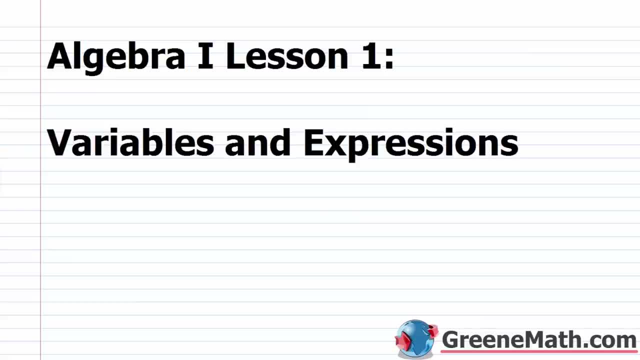 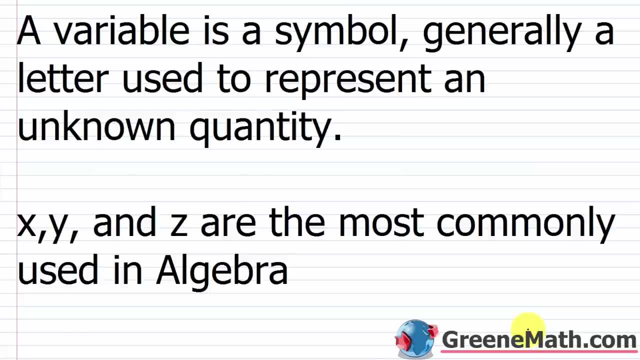 Hello and welcome to Algebra 1 Lesson 1. In this lesson we're going to learn about variables and expressions. So now that we've completed our pre-algebra course and we have a great command over arithmetic, we're going to move on to some tougher material. Now generally when you finish a pre-algebra course or when you first start an Algebra 1 course, you begin learning about something known as a variable. So what a variable is, it's a symbol, generally a letter, and it's going to be a lowercase letter, used to represent an unknown quantity. Another way you can kind of think about this, it's going to be a placeholder. So I put here that x, y, and z are the most commonly used in algebra. But you can use any lowercase letter that you want. Just for right now, these are the ones that you're pretty much going to work with. 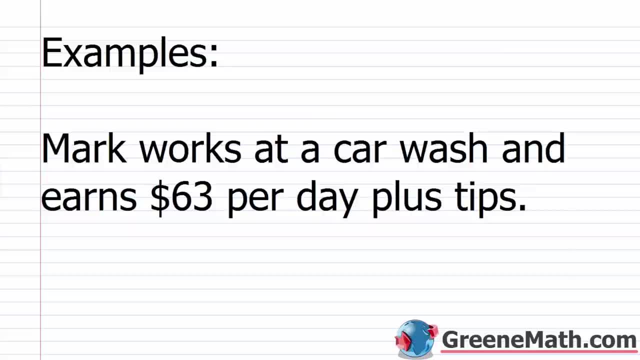 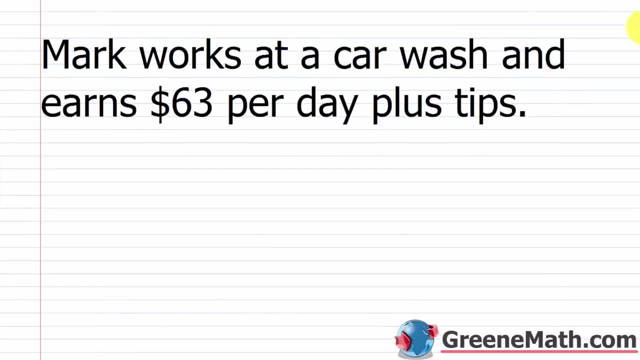 x, y, and z. All right, so here's some examples. So Mark works at a car wash and earns $63 per day plus tips. So if I wanted to kind of model this mathematically and say, how much does he earn every day? Well, I know that he earns $63 at minimum, right? $63 per day. So let me start by putting $63 down. Now we have an additional amount. We have this keyword here that says plus, and then we have tips. We don't know what the amount of tips is going to be, right? Just like a waiter or anybody who works in the service industry that gets tips. You don't know what you're going to get in tips that day. You might get a customer that overly tips or a customer that under tips. So that amount's going to vary. So we can represent this unknown with a variable. So I'd put $63 plus, and let's use the common variable. 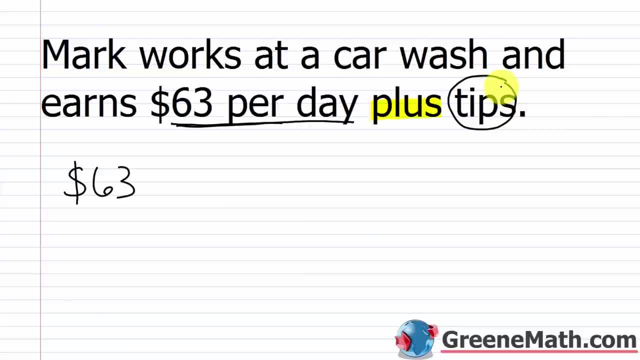 a waiter or anybody who works in the service industry that gets tips. You don't know what you're going to get in tips that day. You might get a customer that overly tips or a customer that under tips, So that amount's going to vary. So we can represent this unknown with a variable. 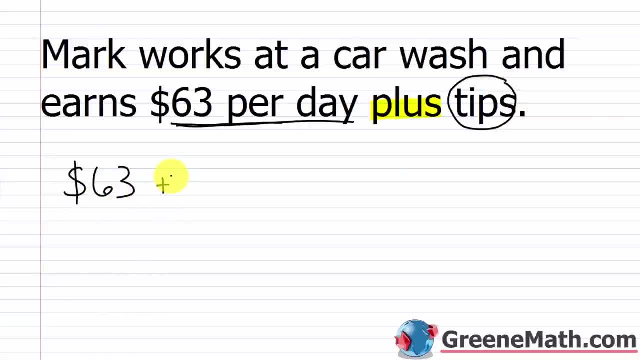 So I'd put $63 plus and let's use the common variable Of X, So plus X, So this represents the amount, the amount of tips. Now we can use this to model what this person, Mark, is going to receive every day. He gets $63 plus X, where X equals the amount. 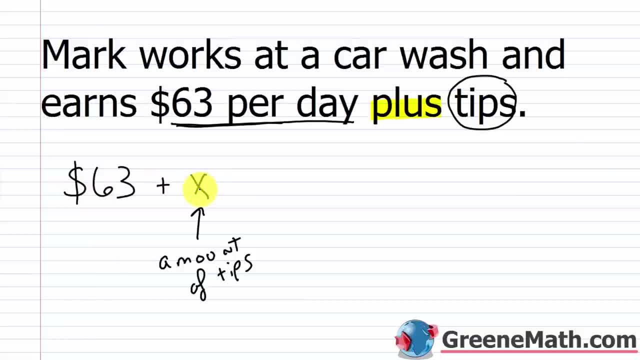 of tips that he's going to receive. So let's say the day is over and he knows that he got $63 plus seven dollars in tips. So X in this case would equal seven. If I want to know how much he made for that day, all I would do is I would take this right here, this seven, and I would plug it. 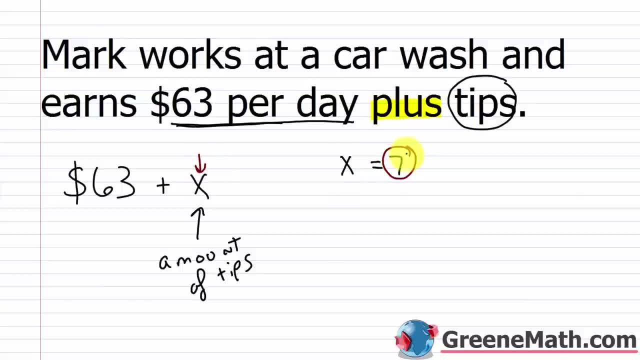 into the X right here, because X equals seven. He got $7 in tips. X was the amount of unknown tips he was going to get, And so we plug in a seven for X and we'd end up with $63 plus seven, and I'll put. 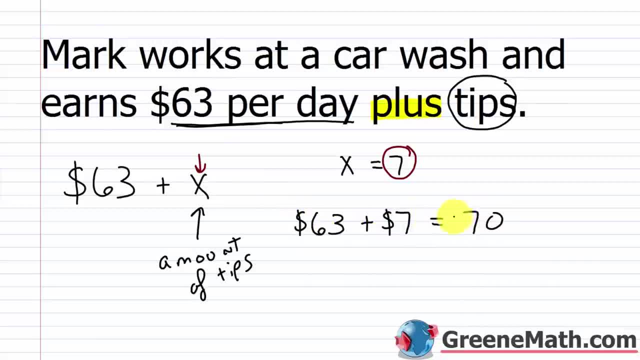 dollars there, just to be consistent. And this will equal $70,. right, That's how much he received for that day, But the next day it's going to be different. So let's say, the next day X is going to equal nine. Well then, I'd take 63 and I'd add nine to that. right, I'd make two more dollars. 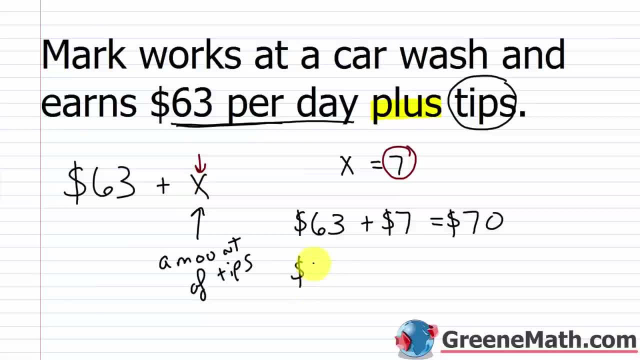 or I'd have 72. So the following day you would have $63 plus. and let me do this in a different color so we don't get confused. nine dollars, right? So in that case X is equal to seven. So we see that as we change the value for X, the value is going to change In this case. 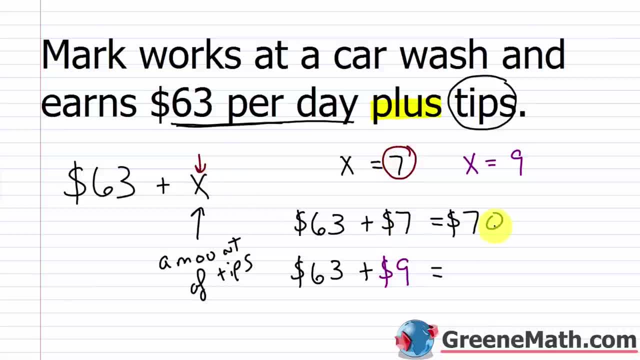 X is equal to seven. I plug in a seven for X and I get 70, right? 63 plus seven is 70. In the other case, X equals nine. So I plug a nine in for X. 63 plus nine is going to give me 72. So he earns. 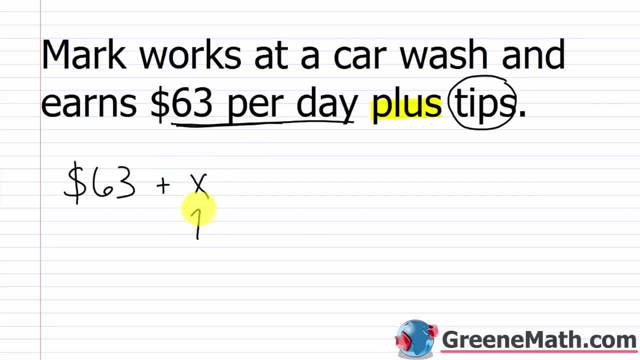 Of X. So plus X. So this represents the amount, the amount of tips. Now we can use this to model what this person Mark is going to receive every day. He gets $63 plus X where X equals the amount of tips that he's going to receive. So let's say the day is over and he knows that he got $7 in tips. So X in this case would equal seven. If I want to know how much he made for that day, all I would do is I would take this right here, this seven, and I would plug it into the X right here because X equals seven. He got $7 in tips. X was the amount of unknown tips he was going to get. And so we plug in a seven for X and we'd end up with $63 plus seven. And I'll put dollars there. just to be consistent. And this will equal $70, right? That's how much he received for that day. But the next day, it's going to be different. So let's say the next day, X is going to equal nine. Well, then I take 63 and I'd add nine to that, right? I'd make two more dollars or I'd have 72. So the following day, you would have $63 plus, and let me do this in a different color so we don't get confused, $9, right? So in that case, X is equal to nine. So we see that as we change the value for X, the value is going to change. In this case, X is equal to seven. I plug in a seven for X and I get 70, right? 63 plus seven is 70. And the other case, X equals nine. So I plug a nine in for X, 63 plus nine is going to give me 72. So he earns $72 in this case. 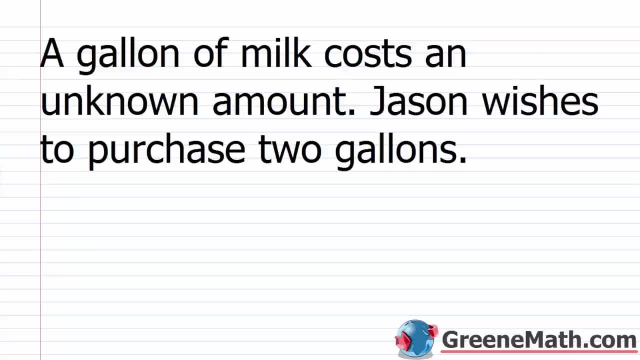 $72 in this case. Let's take a look at another one in case you're a little confused. So a gallon of water costs an unknown amount. Jason wishes to purchase two gallons. Well, again, we can use a variable to model this situation. So I know that he's going to buy two gallons, So that's two. 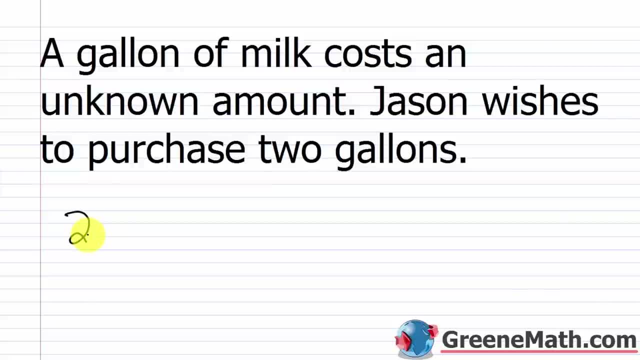 And it costs an unknown amount. So I can use a variable. Let's use Y in this scenario to represent that. So I need to multiply the cost per gallon times the number of gallons. The number of gallons is two. The cost per gallon is unknown, So I would have two times Y. 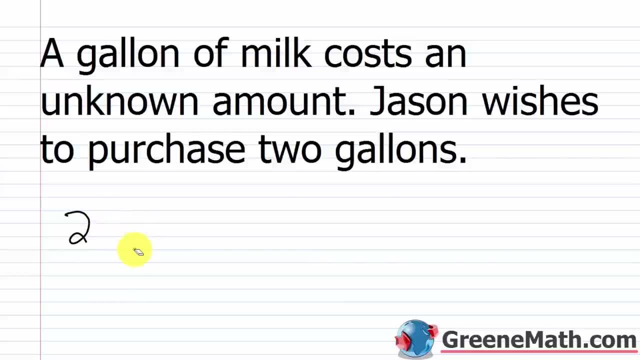 which we're going to write as just two Y. When a number is next to a variable, it implies multiplication. So two Y like that is telling me that I have two times Y or two times Y. You remember back in pre-algebra when I said we stopped using this symbol to imply multiplication? 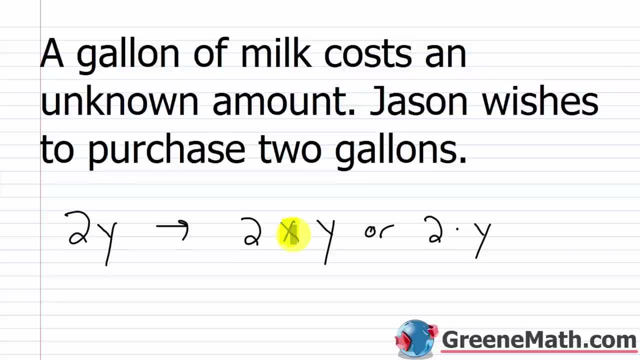 And the reason is because it often gets confused with the variable X. So we'll either use this parentheses or replace the number next to the variable, And this is the most common. You'll just have two times Y like this, just two Y. That implies multiplication. Now if I give you a cost, 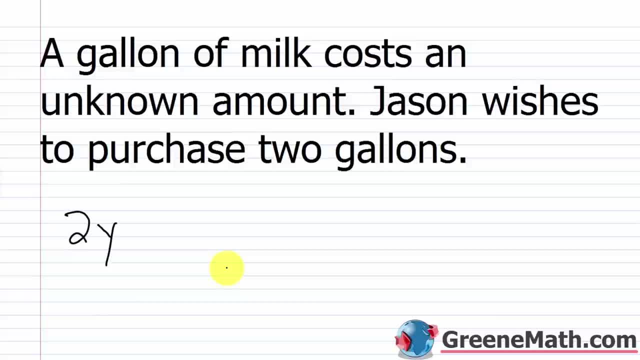 per gallon of milk. I can tell you how much Jason's going to spend on his milk purchase. right, If I say that Y is equal to $1, and I'm not going to put the dollar symbol in this time, I'm just going to put one. Well then, really, all I'm going to do is plug a one in for Y. 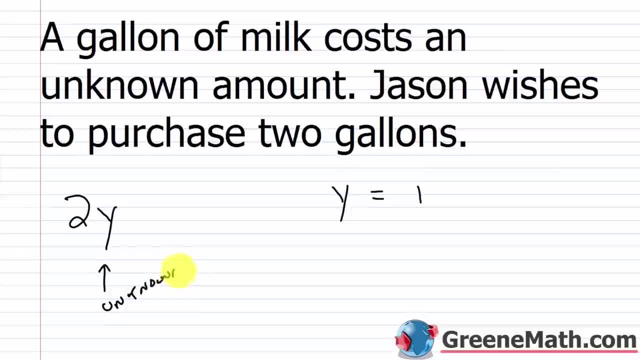 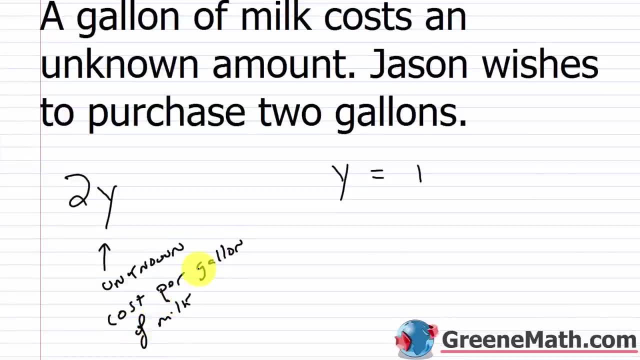 Right, This is the unknown, the unknown cost per gallon of milk. If I tell you that it equals $1, I could just plug a one in there and I can say, okay, well, two times one is two, So two times one is two, So he spends $2 on two gallons of milk. If that amount changes, right? If it. 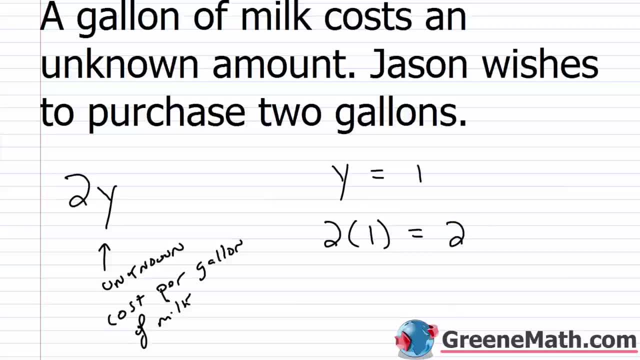 changes if I say: well, the price of milk just went up, So let's say that now Y is going to be equal to three. Okay, We had a big price increase. Well, now I'm going to plug in a three for Y, So instead of two, 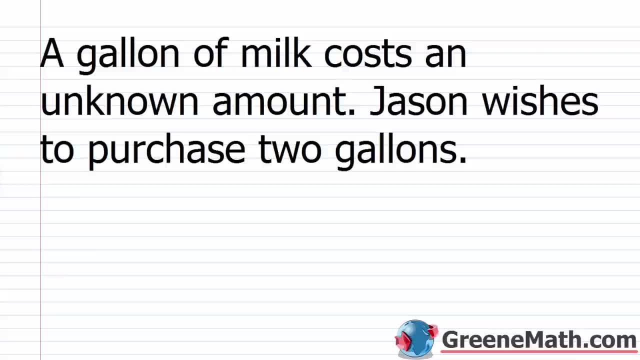 Let's take a look at another one in case you're a little confused. So a gallon of milk costs an unknown amount. Jason wishes to purchase two gallons. Well, again, we can use a variable to model this situation. So I know that he's going to buy two gallons. So that's two. And it costs an unknown amount. So I can use a variable. Let's use Y in this scenario to represent that. So I need to multiply the cost per gallon times the number of gallons. The number of gallons... is 2 the cost per gallon is unknown so I would have 2 times Y which we're gonna write as just 2y okay when a number is next to a variable it implies multiplication so 2y like that is telling me that I have 2 times Y or 2 times Y you remember back in pre-algebra when I said we stopped using this symbol to imply a multiplication and the reason is because it often gets confused with the variable X so we'll either use this symbol or we'll use parentheses or replace the number next to the variable and this is the most common you'll just have 2 times Y like this just 2y that implies multiplication now if I give you a cost per gallon of milk I can tell you how much Jason's gonna spend on his 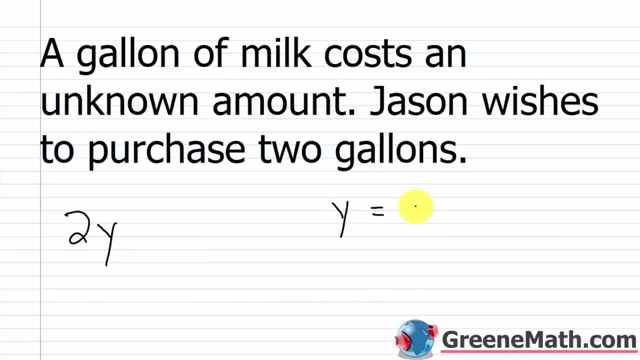 milk purchase right if I say that Y is equal to $1 and that's $1 and that's the cost per gallon of milk I can tell you how much Jason's gonna spend on his milk purchase right if I say that Y is equal to $1 and and I'm not gonna put the dollar symbol in this time, I'm just gonna put one. Well, then really all I'm gonna do is plug a one in for y, right? 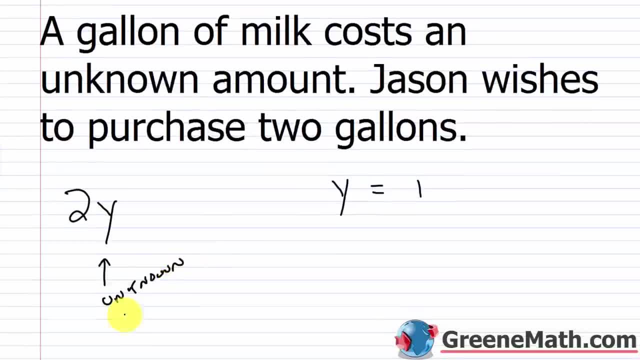 This is the unknown cost per gallon of milk. 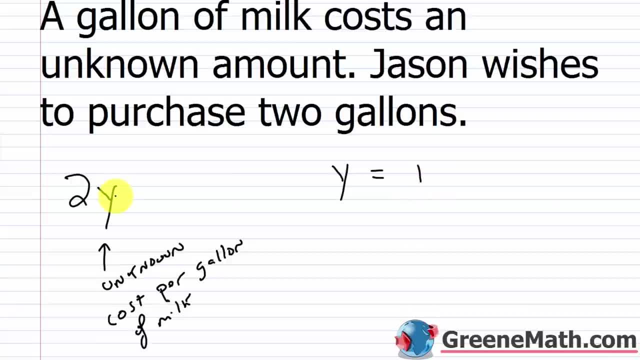 If I tell you that it equals $1, I could just plug a one in there, and I could say, okay, well, two times one is two. 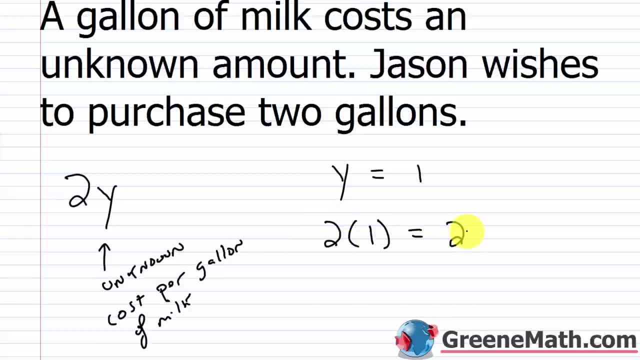 So two times one is two. 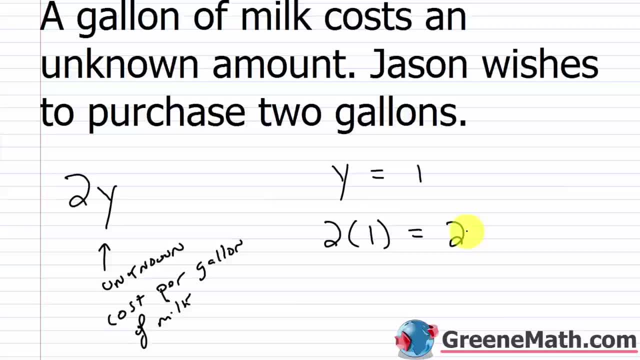 So he spends $2 on two gallons of milk. If that amount changes, right? If it changes, if I say, 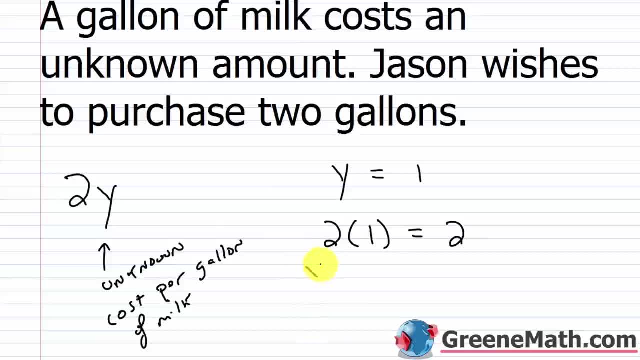 well, the price of milk just went up. So let's say that now y is gonna be equal to three, okay? We had a big price increase. Well, now I'm gonna plug in a three for y. So instead of two times one, I would have two times three, and that's gonna give me six. 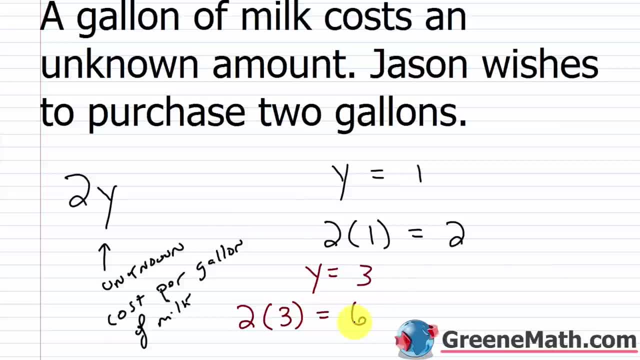 So now he's gonna spend $6 on two gallons of milk. And that makes sense. 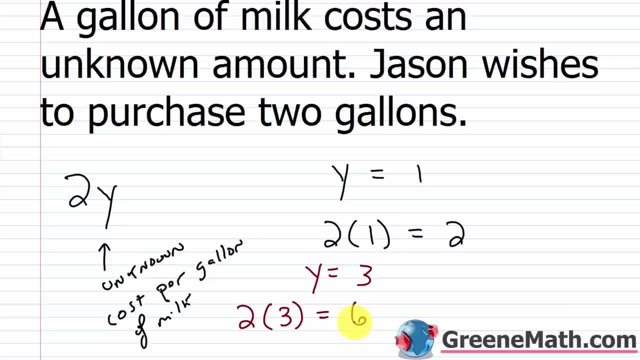 Two times three is six. So if Jason buys two gallons of milk at $3 per gallon, he spends $6. 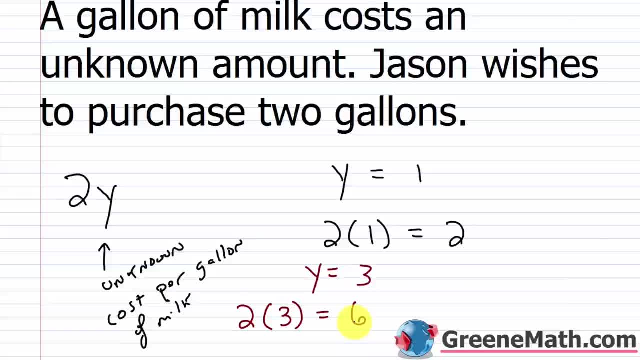 In the other scenario, if he buys two gallons of milk at $1 a gallon, he's gonna spend $2. 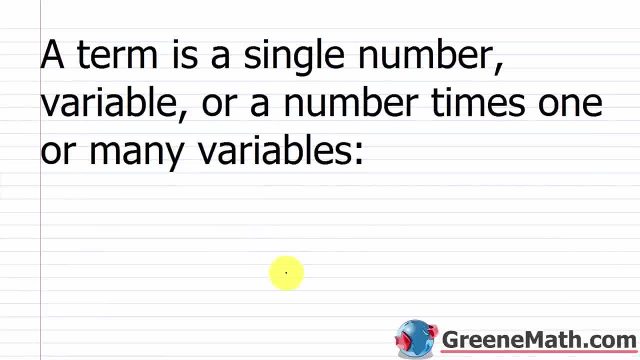 All right, so let's get into some more kind of definitions. 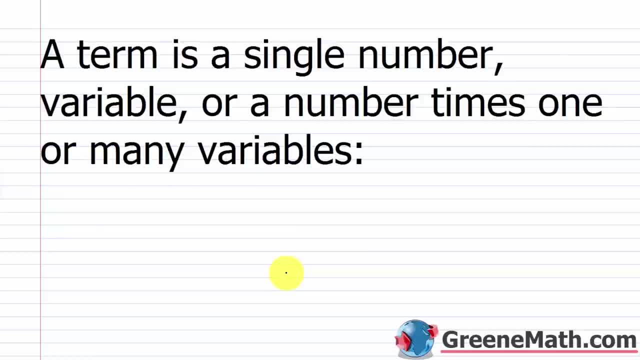 A term is a single number, variable, or a number times one or many variables. 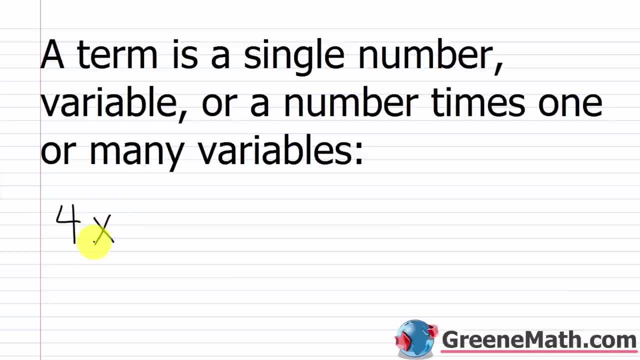 So for example, you might see something like forex. That's a term. 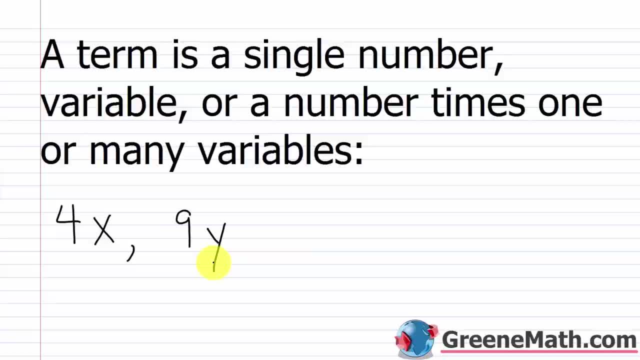 Or you might see something like nine y. That's a term. 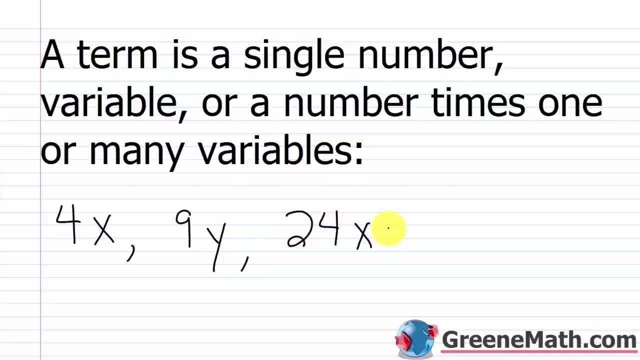 Or you might see something like 24 x y z. 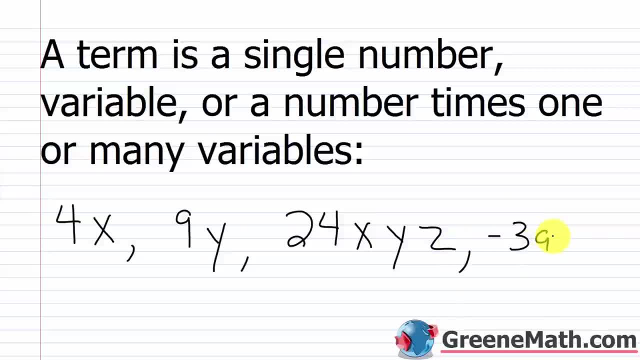 Or you might see something like negative three a. These are all examples of a term, right? A single term. 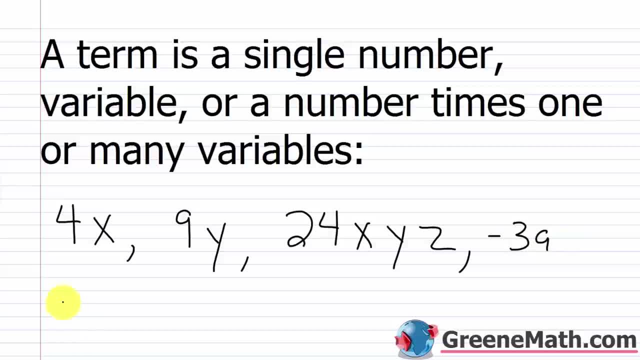 Again, it's a number by itself. So if I just had, let's say the number seven, that's a term. 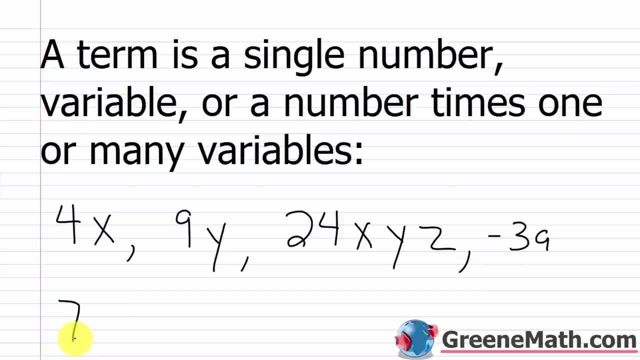 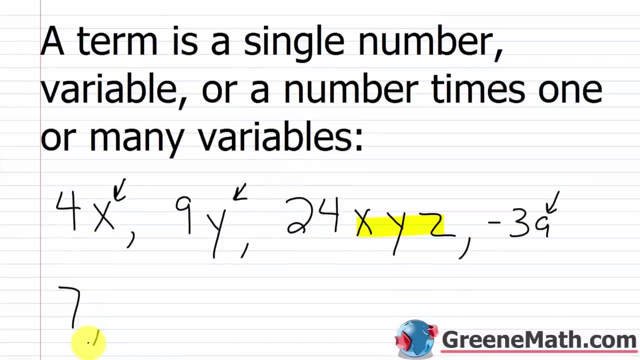 Or it's a number times one or many variables. So in this case, you have one variable, one variable, one variable. In this case, you have many variables. And these variables can be raised to powers. So for example, I could have had an example of a term 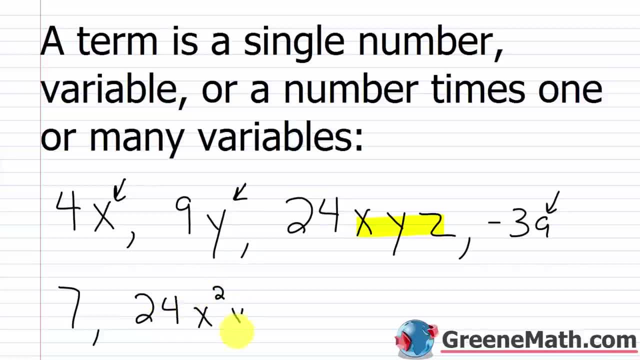 where I have 24 x squared y to the fourth, 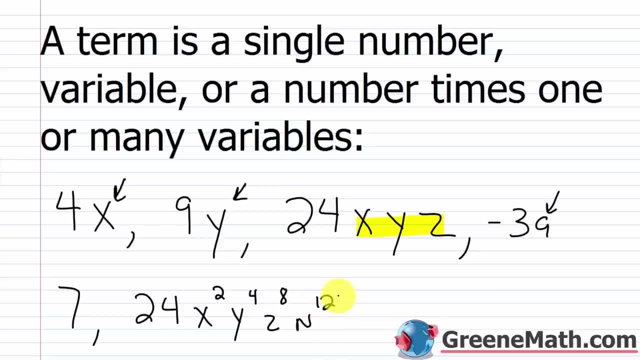 z to the eighth, let's say n to the 12th. That's a term, right? A single term. 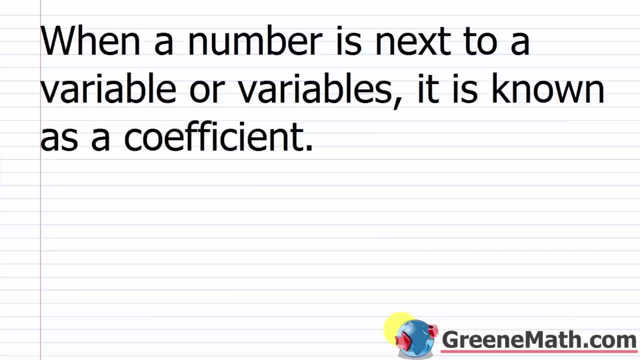 Now here's another kind of definition thing. When a number is next to a variable, or a number, a variable or variables, it is known as a coefficient. 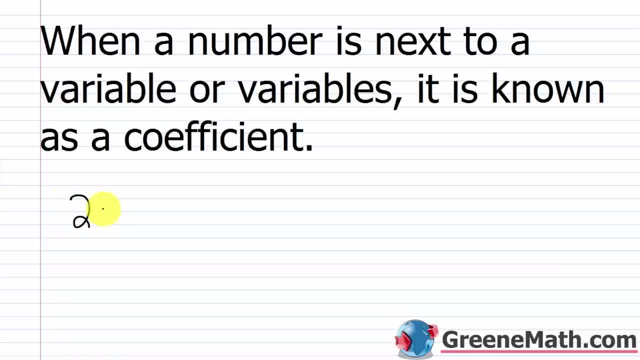 So in all these scenarios where I'm saying, okay, two times y, right? Two y is how we would say it. 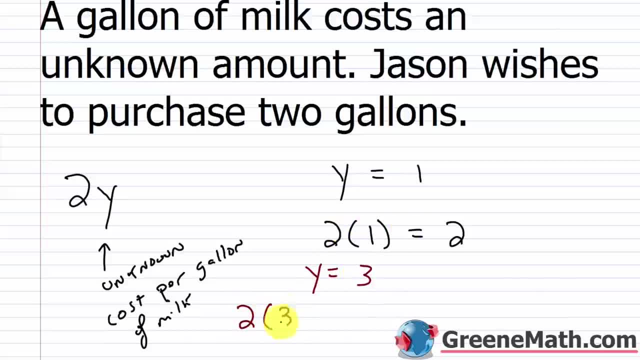 times one, I would have two times three and that's going to give me six. So now he's going to spend $6 on two gallons of milk. right, And that makes sense. Two times three is six. So if Jason buys two gallons of milk at $3 per gallon, he spends $6.. In the other scenario, 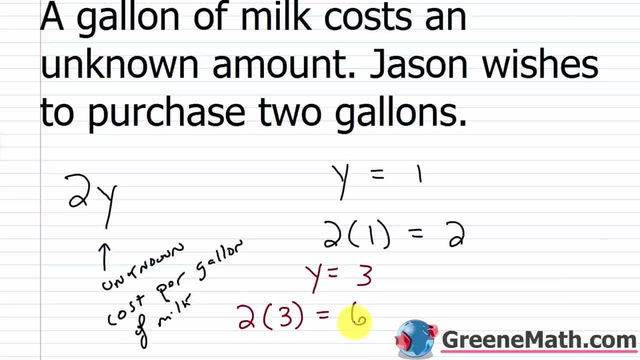 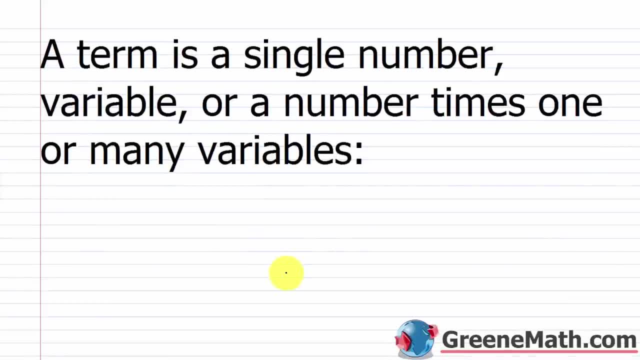 if he buys two gallons of milk at $1 a gallon, he's going to spend $2.. All right, So let's get into some more kind of definitions. A term is a single number variable or a number times one or many variables. So, for example, you might see something like 4X. Hey, that's a term. 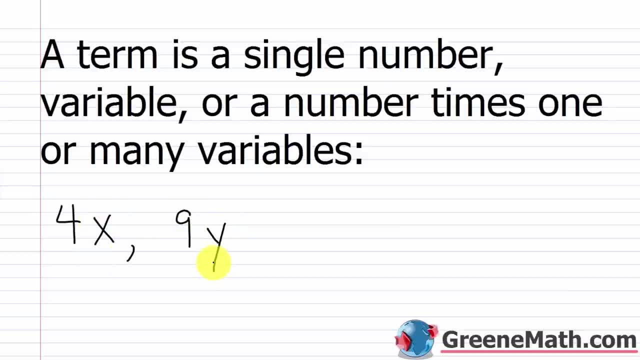 Or you might see something like 9Y- That's a term- Or you might see something like 24X Y Z. Or you might see something like negative 3A. These are all examples of a term right A. 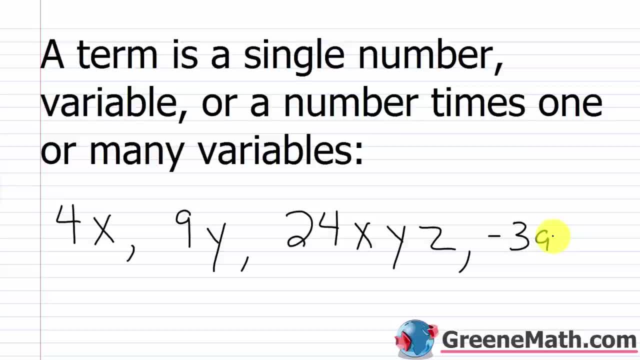 single term, Again it's a number by itself. So if I just had, let's say, the number seven, that's a term, Or it's a number times one or many variables. So in this case you have one variable, one variable, one variable. In this case you have many variables And these variables. 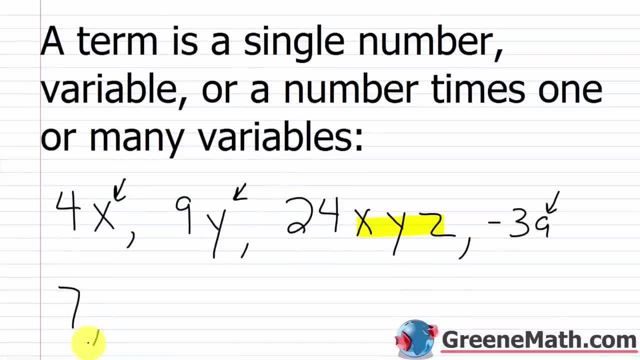 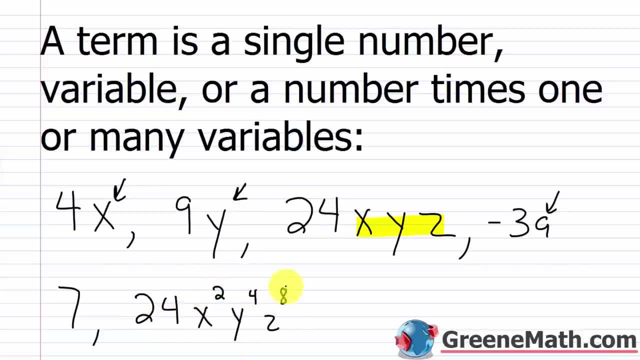 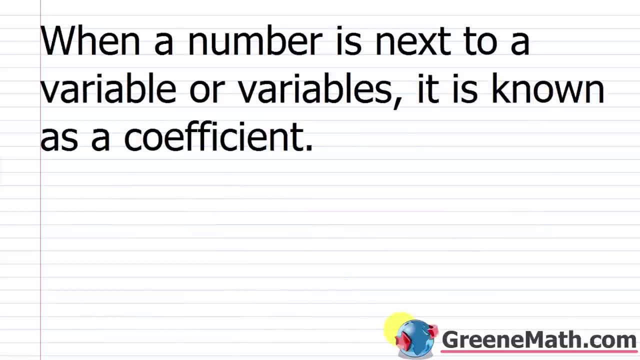 squared: Y to the fourth, Z to the eighth, let's say N to the 12th. That's a term, right, A single term. Now here's another kind of definition thing, When a number is next to a variable or variables. 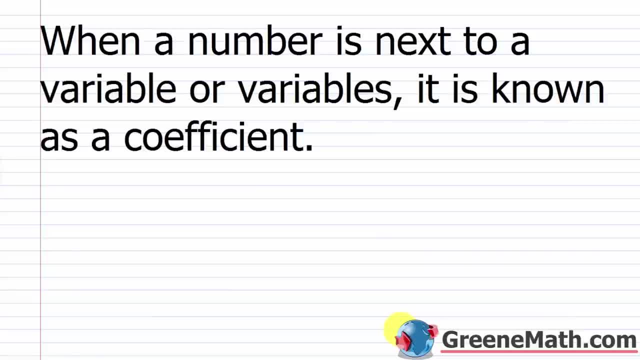 it is known as a coefficient. So in all these scenarios where I'm saying, okay, two times Y, right, Two Y is how we would say it, but two times Y really, because it's multiplying. Two is the number that's multiplying the variable Y. It's known as a coefficient. 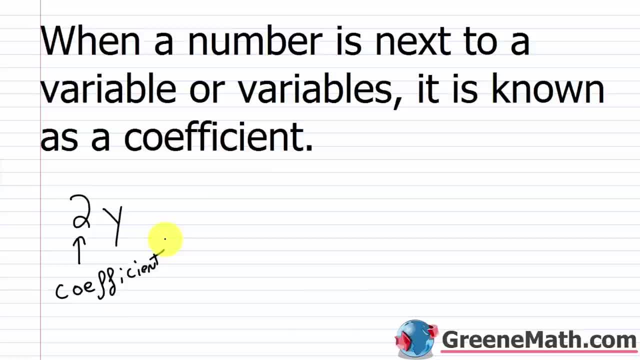 Two is the coefficient of Y. If I had, let's say, four X squared Z, four is the coefficient right. It's the number that's multiplying the variable Y. So in this case it's known as a coefficient. So in all these scenarios where I'm 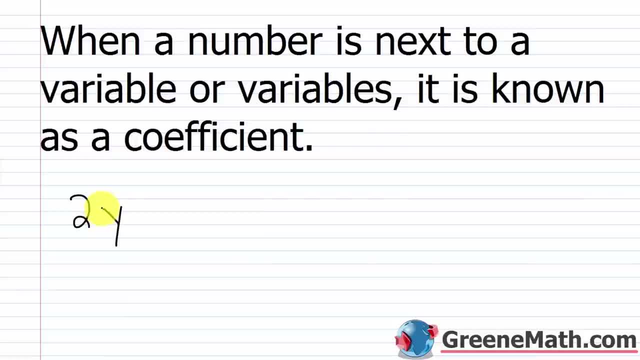 But two times y, really, because it's multiplying. Two is the number that's multiplying the variable y. It's known as a coefficient. 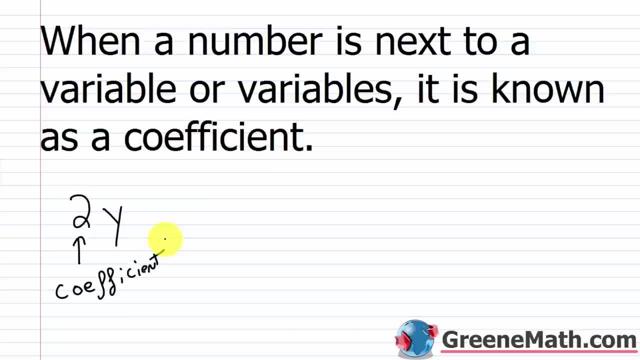 Two is the coefficient of y. If I had, let's say, two times y. 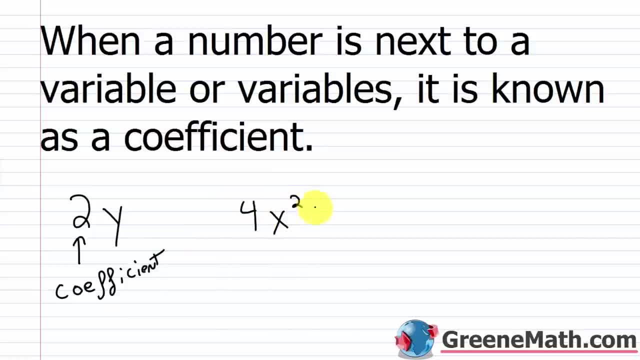 Let's say four x squared z. 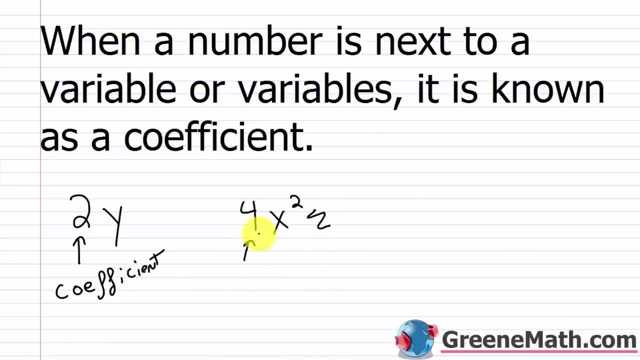 Four is the coefficient, right? It's the number that's multiplying the variable, or again, variables if you have more than one. So this is again, a coefficient. 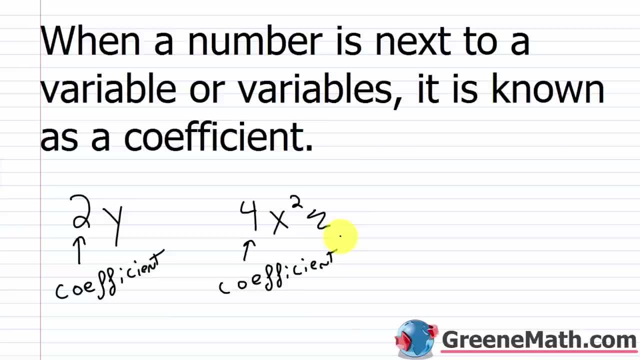 And these are kind of very basic definitions that even if you don't get them in this video, you can write them down and put them on flashcards if you want. We're gonna talk about them over and over and over again. By the time you get to the 10th lesson, you will know all of these terms, right? It won't be an issue for you. 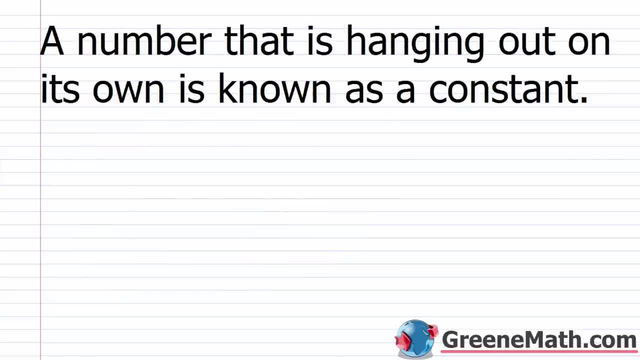 All right, so a number that is hanging out on its own is known as a constant. 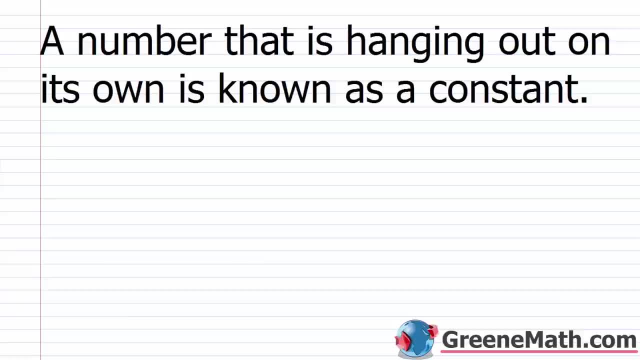 So you're gonna get to a point in this lesson where we start talking about algebraic expressions, and you might see something that looks like five x plus seven. 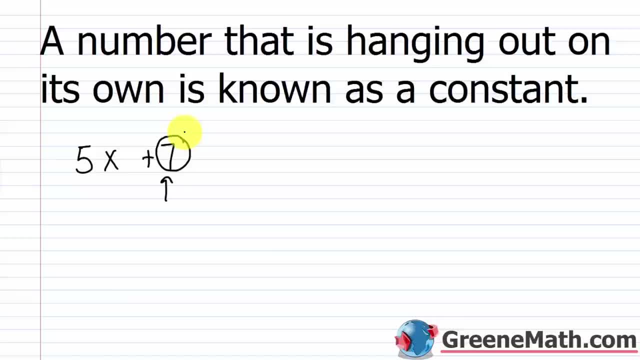 So this number, this seven that's hanging out by itself, is a constant. This is a constant. Its value is not gonna change. 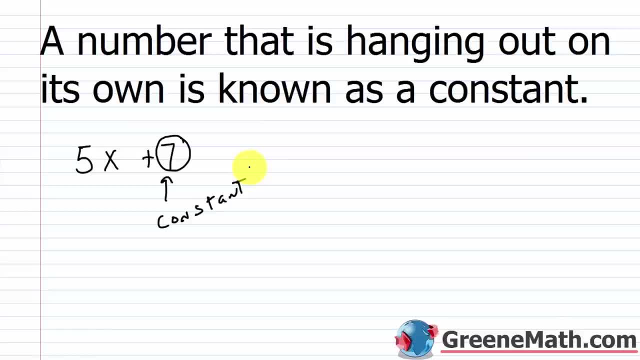 It's what we've worked with in pre-algebra, right? Where we're just doing basic operations. If I do seven times three, that value is always gonna be 21, right? It's not gonna change because we're working with constants. If I have five x plus seven, well, I don't know what the value of x is. Again, it's allowed to vary, it's allowed to change. And so the value for this is going to change based on what x is. 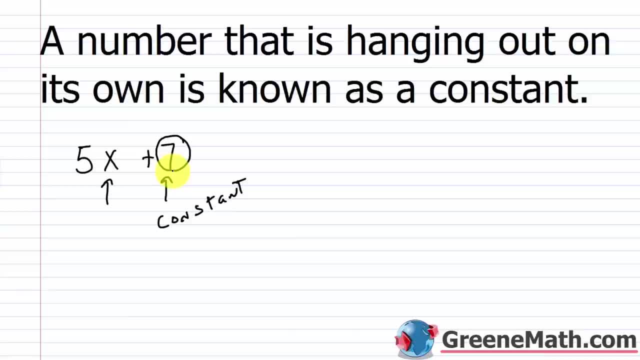 If I change x, I change the value of this whole algebraic, algebraic expression. So that's kind of the difference here. 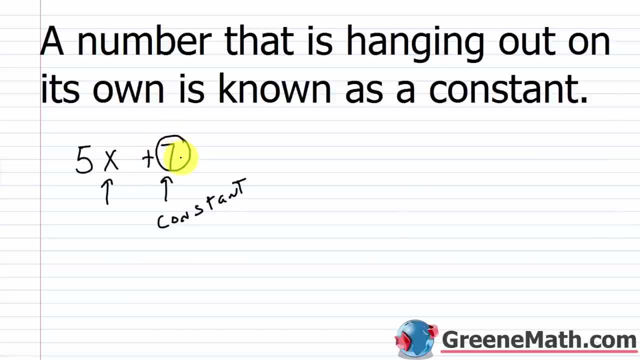 That's why we say this is a constant, because the number seven is not gonna change. 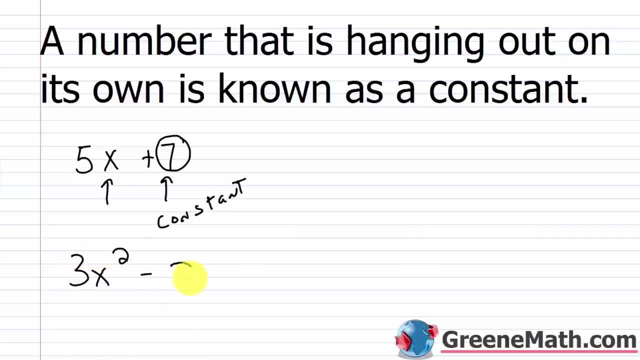 If I have something like three x squared minus two. Two is hanging out by itself. Two's value is constant, it's not gonna change. 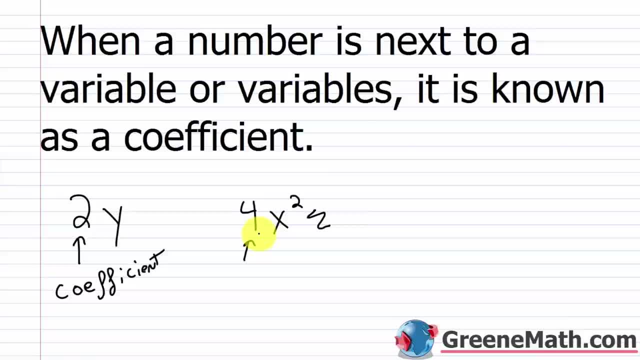 variable, or again variables if you have more than one. so this is again a coefficient and these are kind of very basic definitions that even if you don't get them in this video, you can write them down and put them on flashcards if you want. we're gonna talk about them over and over and over again. by the time, 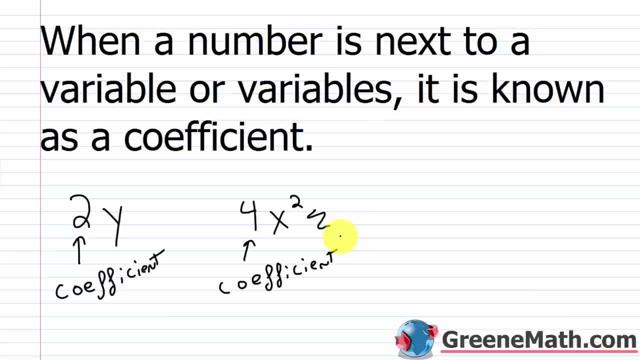 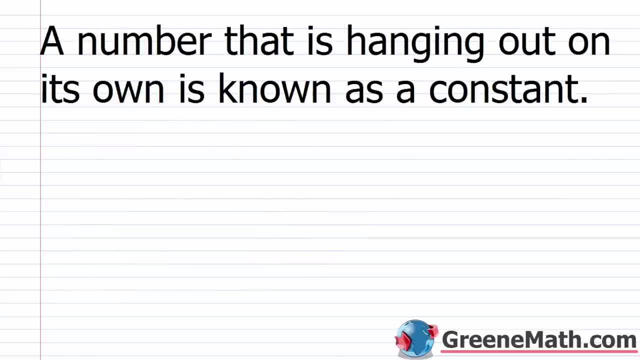 you get to the tenth lesson, you will know all of these terms, right? it won't be an issue for you, all, right? so a number that is hanging out on its own is known as a constant. so you're gonna get to a point in this lesson where we start. 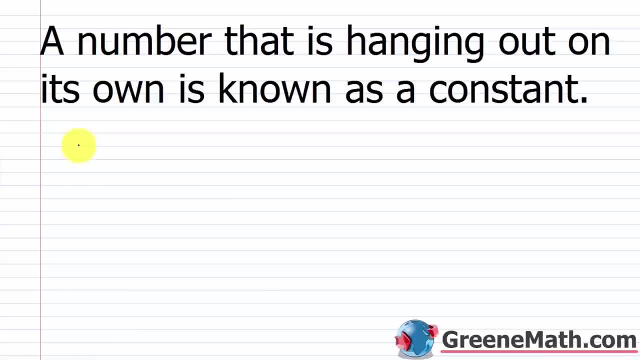 talking about algebraic expressions and you might see something that looks like 5x plus 7. so this number, this 7 that's hanging out by itself, is a constant. this is a constant. its value is not going to change. it's what we've worked with in. 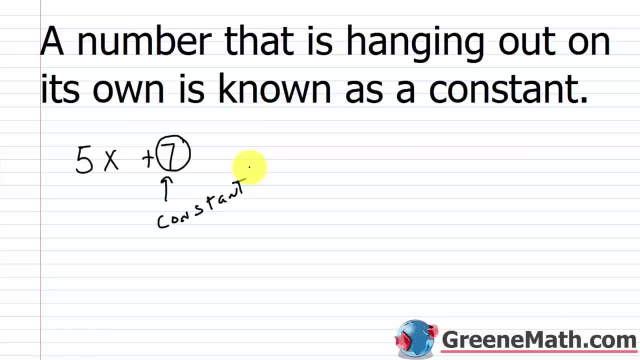 pre-algebra, right, where we're just doing basic operations. if I do 7 times 3, that value is always going to be 21, right? it's not going to change because we're working with constants. if I have 5x plus 7, well, I don't know what the value. 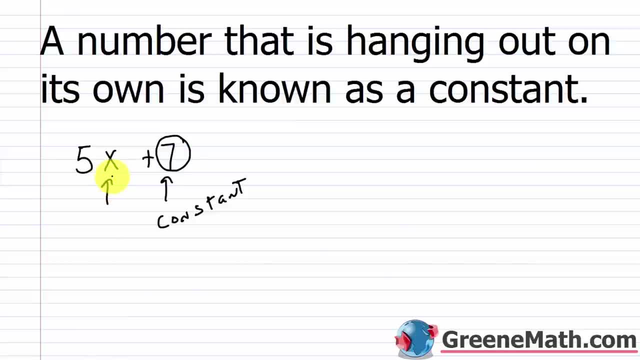 of X is, again, it's allowed to vary, it's allowed to change, and so the value for this is going to change based on what X is. if I change X, I change the value of this whole algebraic expression. so that's kind of the difference here. 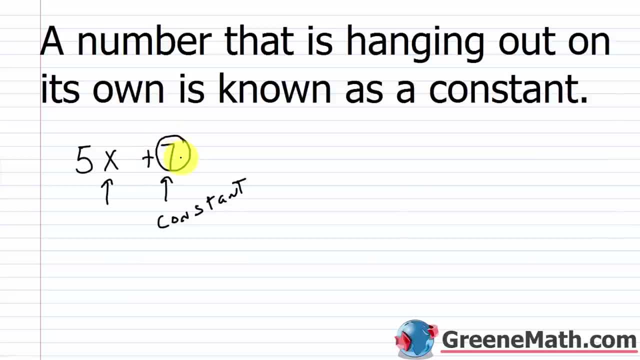 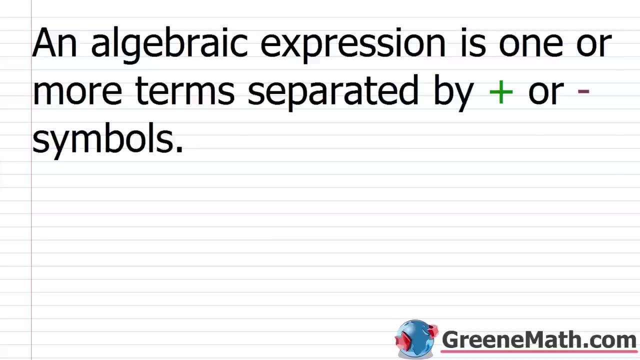 that's why we say this is a constant, because the number 7 is not going to change over and over again. but this leaves us with this very important definition, which is 100% safe. so as we start talking about algebraic terms, we kind of have to appreciate the benefits or the advantages to an algebraic 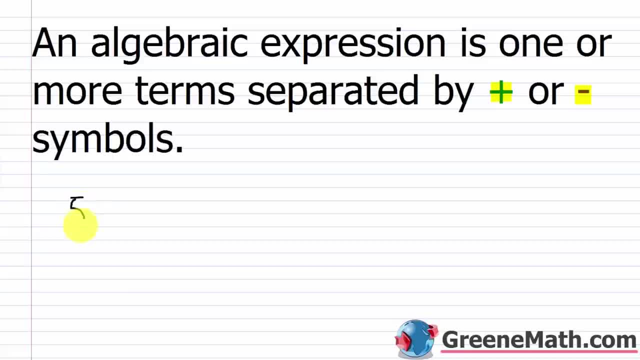 expression. look at an example. Let's say we have something like 5x plus 2y minus 4z. So if you want to look at that algebraic expression and say where are the individual terms, Well, every time you see. 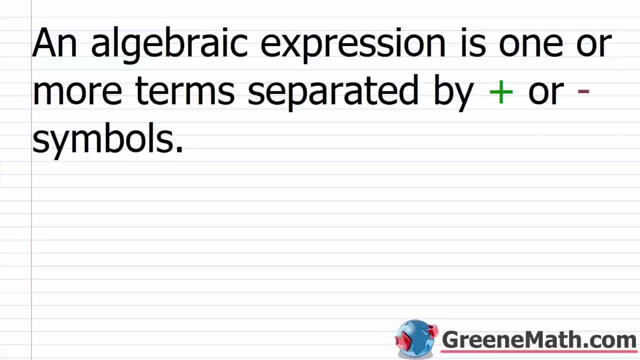 So that's why we refer to it again as a constant. 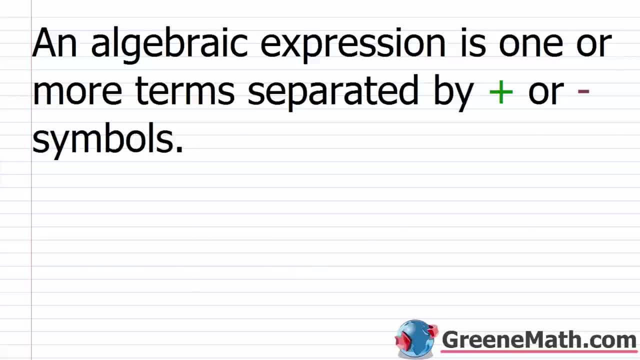 All right, so here's a pretty important definition. An algebraic expression is one or more terms separated by plus or minus symbols. 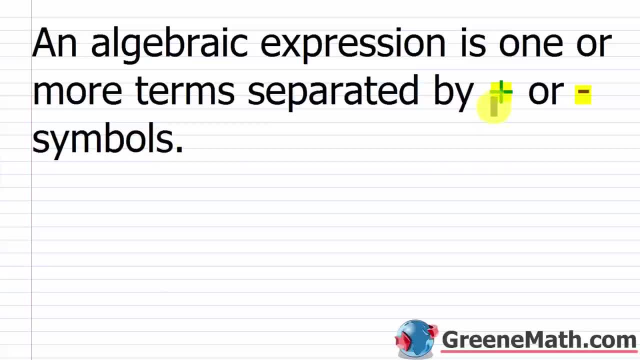 So again, your terms in an algebraic expression are separated by the plus and minus symbols. Very important. 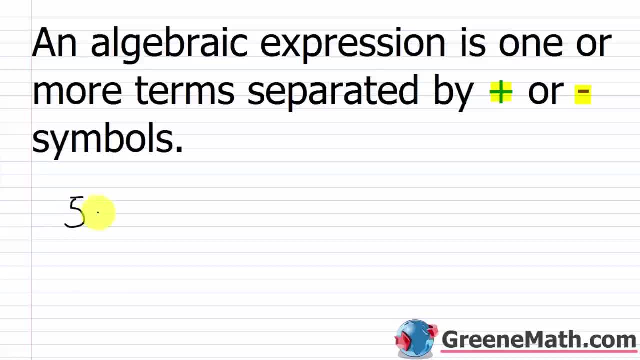 So let's look at an example. Let's say we have something like five x plus two y minus four z. 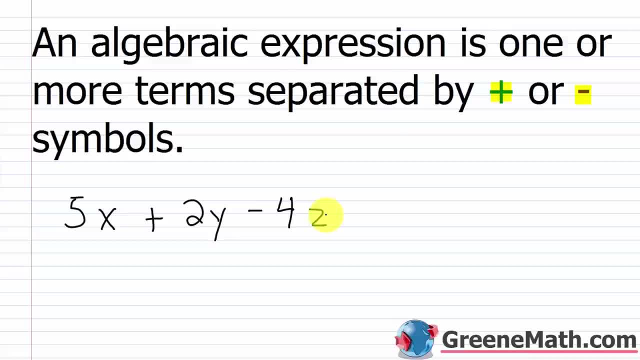 So if you wanna look at that algebraic expression and say, where are the individual terms? Well, every time you see a plus or minus sign, you've cut off a term. 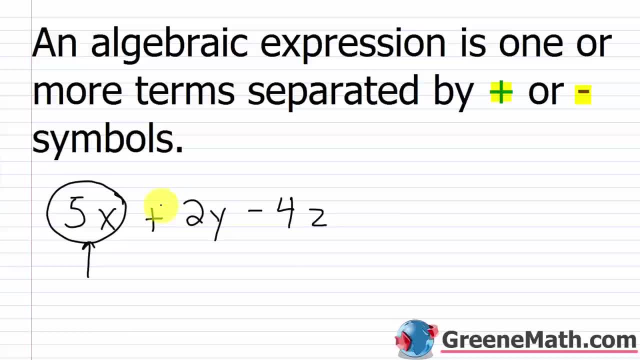 So this is a term. This five x, because there's a plus here, that cuts off this term from this term. 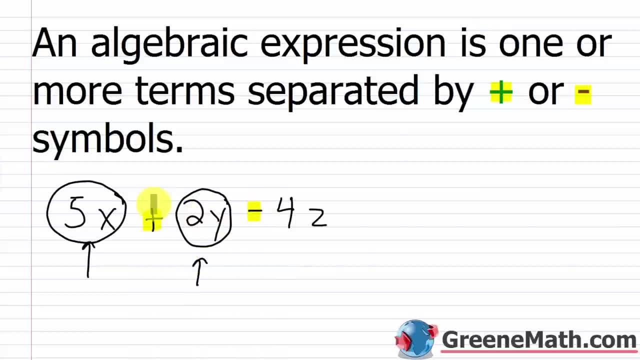 You have a minus sign here, and you have a plus sign over here. So it kinda separates everything. 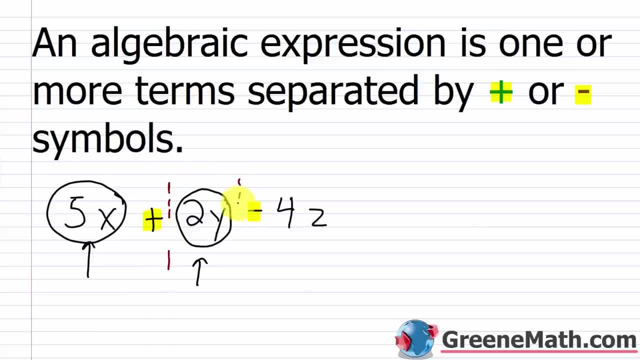 Let me just kinda draw a line here in a different color. This kinda separates everything. 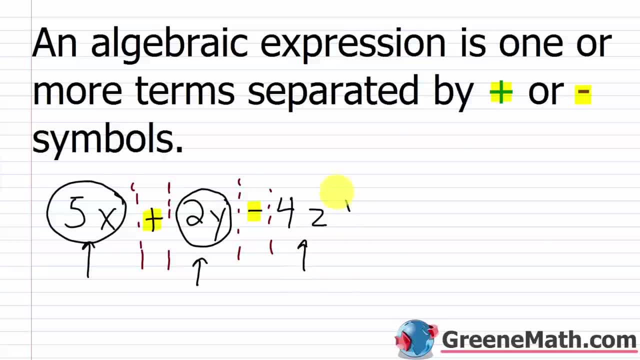 And then here, where you have four z, again, that's a term. 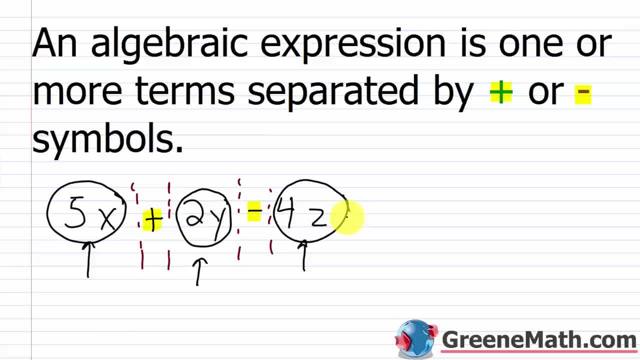 So you have five x, two y, and four z. That make up the terms here. 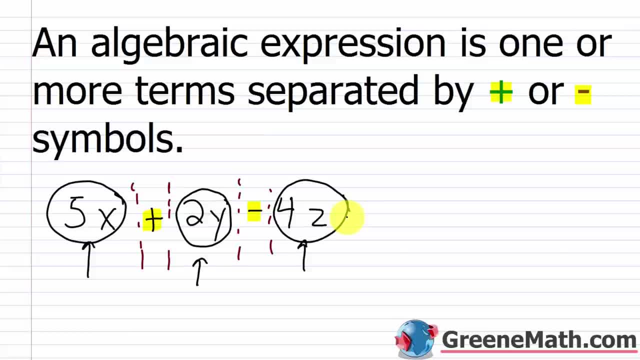 And it's called an algebraic expression because there are variables involved. If you just kinda have numbers involved, we just refer to that as an expression. 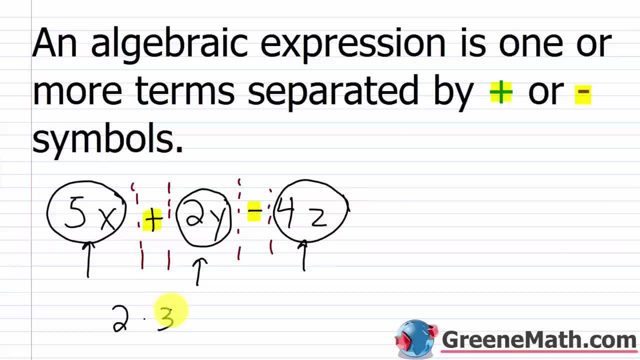 So if you had something like two times three, that's an expression. We work with that in pre-algebra. So two times three is six. 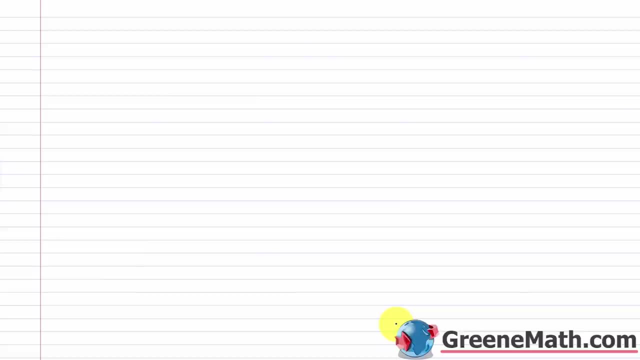 All right, so the main thing about an algebraic expression is that the value will change as its value given for the variables involved are changed. 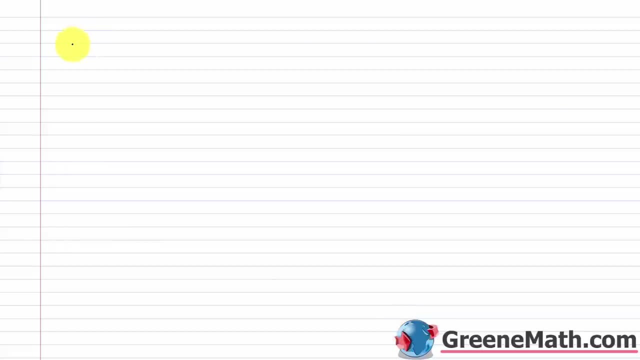 So let me give you some examples. Let's say we had something simple like two x plus three. And I say I wanna let x, let x equal four. 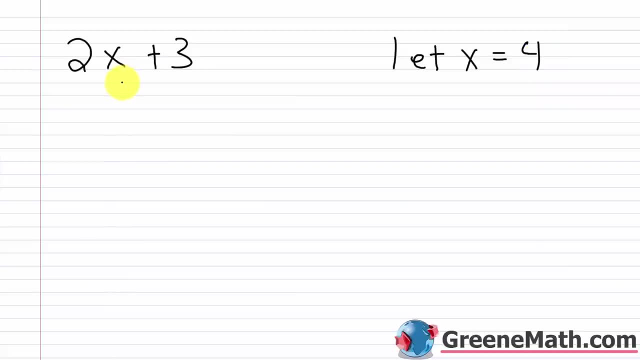 Well, what I'm gonna do is, everywhere I see an x in the algebraic expression, I'm gonna plug in a four. 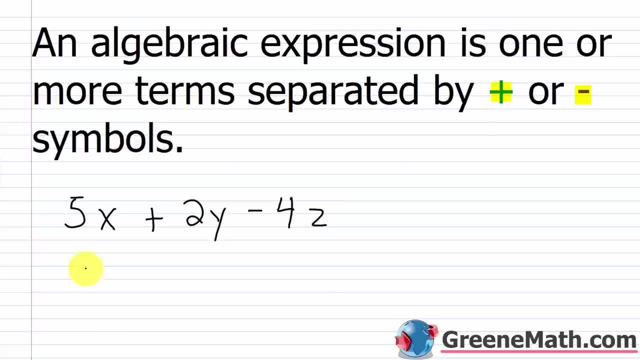 a plus or minus sign, you've cut off a term. So this is a term. this 5x, because there's a plus here, right? That cuts off this term from this term. Then this 2y is a term, right, You have a. 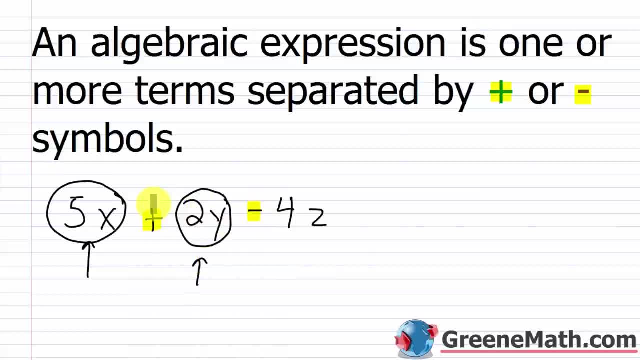 minus sign here and you have a plus sign over here, So it kind of separates everything. Let me just kind of draw a line here in a different color. This kind of separates everything. And then here where you have 4z, again that's a term, So you have 5x, 2y and 4z that make up. 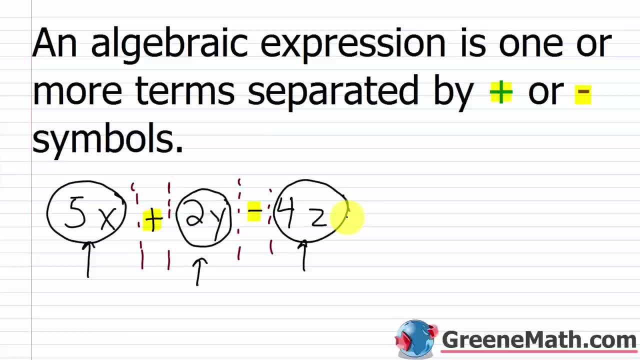 the terms here And it's called an algebraic expression Because there are variables involved. If we just kind of have numbers involved, we just refer to that as an expression, right? So if you had something like you know, 2 times 3, that's an. 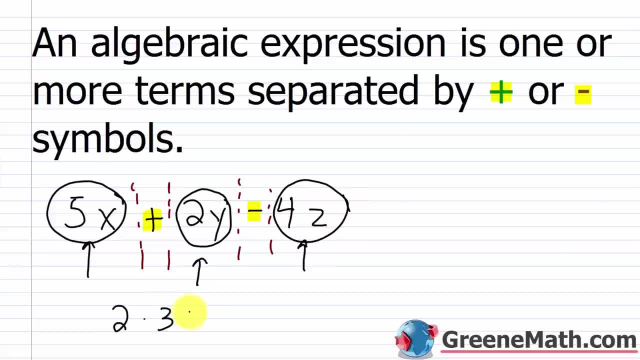 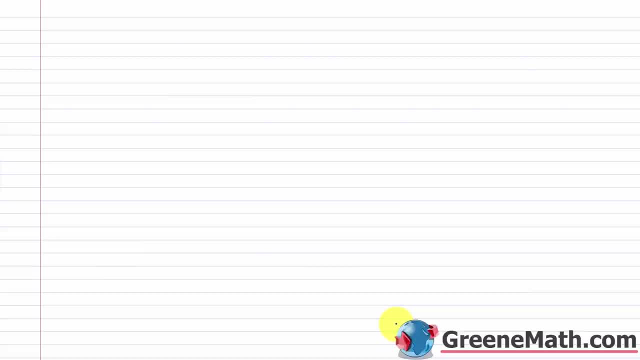 expression right. We work with that in pre-algebra. So 2 times 3 is 6.. All right, so the main thing about an algebraic expression is that the value will change as its value given for the variables involved are changed. So let me give you some examples. Let's say we had something simple like: 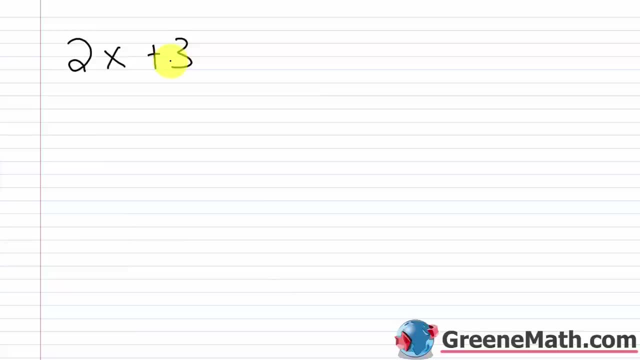 2x plus 3.. And I say I want to let x equal 4.. Well, what I'm going to do is, everywhere I see an x in the algebraic expression, I'm going to plug in a 4.. So I'm going to take this value and plug it. 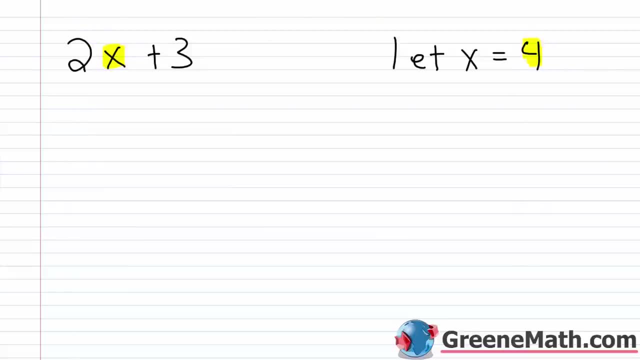 in here, everywhere I see an x, So that means that I'm going to have 2 times 4 plus 3.. And again I can put parentheses around 4 and put it next to 2, and it implies multiplication, Remember. 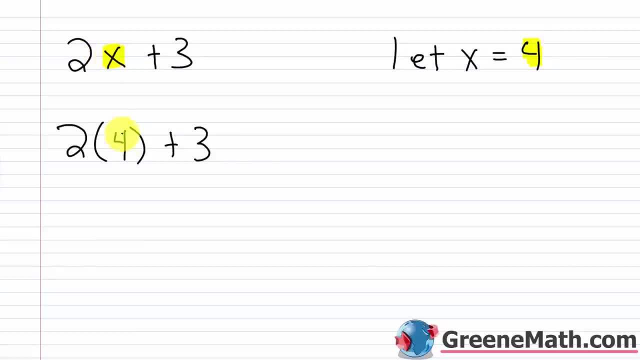 2x is the same as 2 times x. So when I replace x with 4, I'm still going to do the multiplication operation. But now, since it's not a variable, it's a number, that I replaced the variable with. 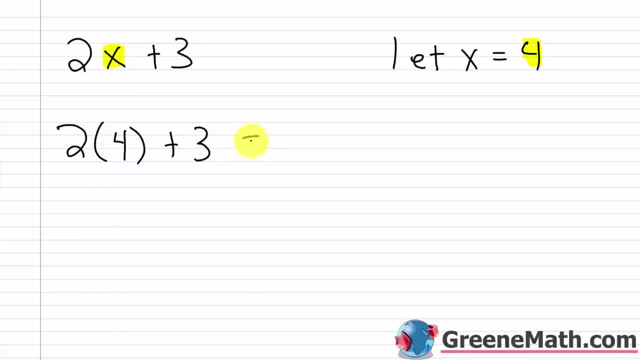 I can just calculate right: 2 times 4 is 8.. So this would be 8 plus 3.. And then 8 plus 3 is 11.. And again, I did the multiplication first because, please excuse my dear Aunt Sally, right, Remember your order of operations. This is where you're. 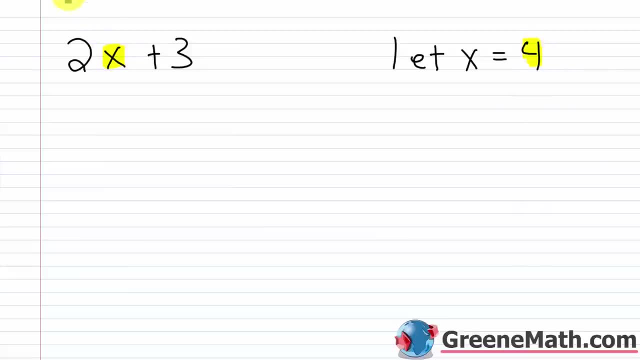 So I'm gonna take this value and plug it in here, everywhere I see an x. So that means that I'm going to have two times four plus three. And again, I can put parentheses around four and put it next to two and it implies multiplication. Remember, two x is the same as two times x. So when I replace x with four, I'm still gonna do the multiplication operation, but now since it's not a variable, it's a number that I replaced the variable with, I can just calculate, right? Two times four is eight. 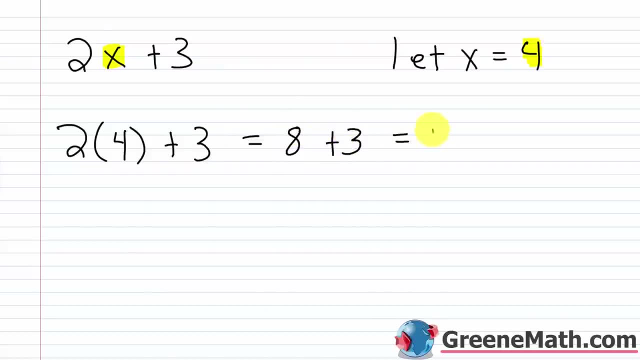 So this would be eight plus three. And then eight plus three is 11. 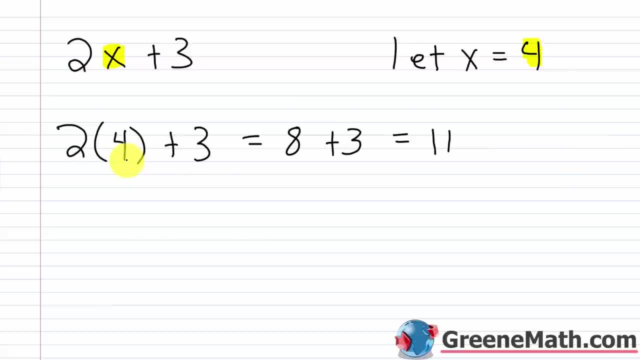 And again, I did the multiplication first because of the, please excuse my dear Aunt Sally, right? Remember your order of operations. This is where you're really gonna use them. All right, so let's say we change the value of x. 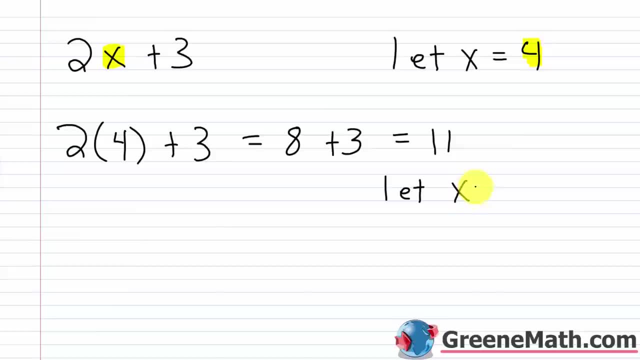 Let's say we wanna let x now equal, I don't know, let's say five. 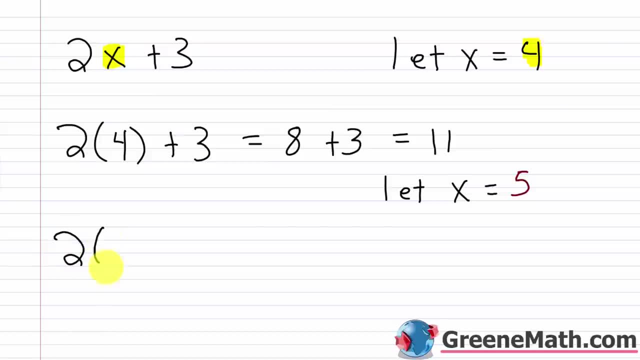 So instead of plugging in a four for x, now I'm gonna say, well, two times five plus three is gonna equal what? Again, I'm plugging in, now I'm gonna say, well, two times five plus three is gonna equal what? Again, I'm plugging in a four for x. Now I'm gonna say, well, two times five plus three is gonna equal what? 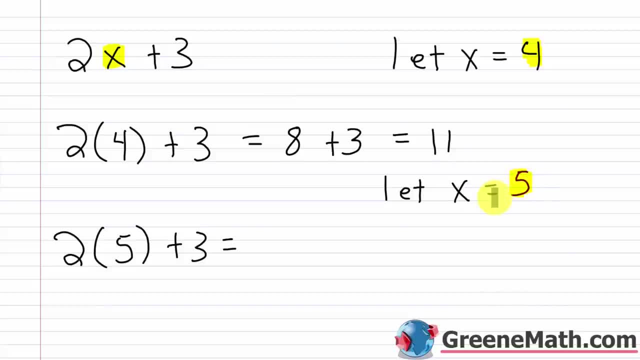 for x whatever value I let x equal. So that's why there's a 5 there. And so we just calculate. 2 times 5 is 10. Then 10 plus 3 is 13. And I did that one step versus 2 up here. Hopefully you can follow, right? 2 times 5 is 10. Then 10 plus 3 again is 13. So as I change the value of x, 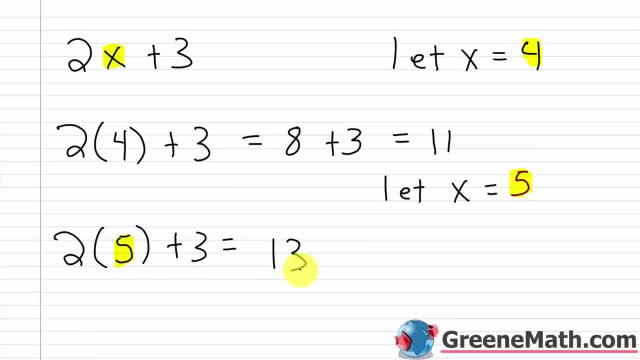 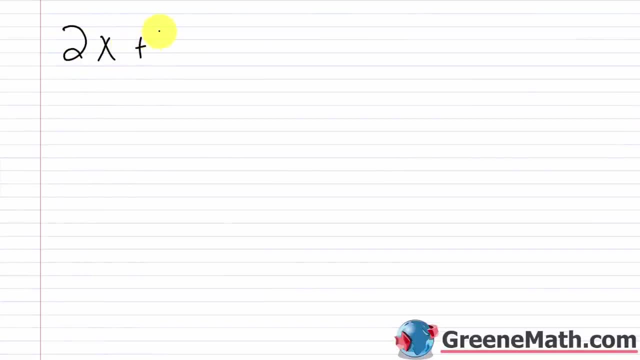 the value of the algebraic expression will change. Let's do one more. Let's say, again, 2x plus 3. Let's let x equal negative 2. So I'm going to plug in a negative 2 for x, 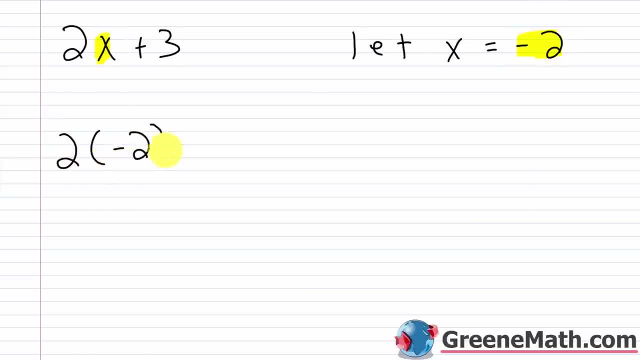 right? Very, very simple. So 2 times negative 2 plus 3 equals what? 2 times negative 2. Remember, positive times negative is negative. 2 times 2 is 4. So that's going to give me negative 4, then plus 3. And at this point, we know how to add integers, right? Negative 4 plus 3 is negative 1. All right. So again, in each case, we got a different value for the algebraic expression because we chose a different 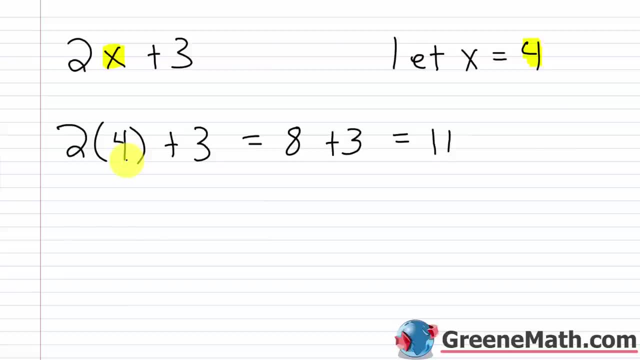 really going to use them. All right. So let's say we change the value of x. Let's say we want to let x now equal- I don't know. let's say 5.. So instead of plugging in a 4 for x now, I'm going to say: 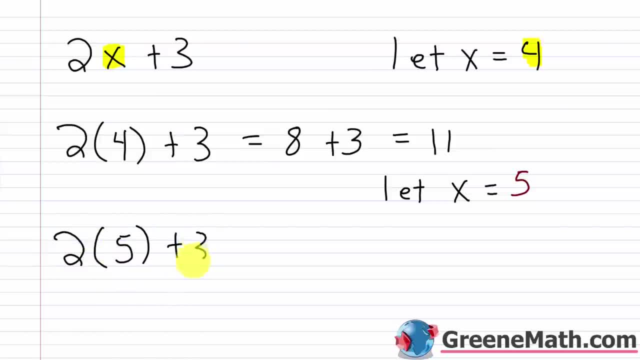 well, 2 times 5 plus 3 is going to equal what? Again, I'm plugging in for x. whatever value I let x equal. So that's why there's a 5 there, And so we just calculate 2. 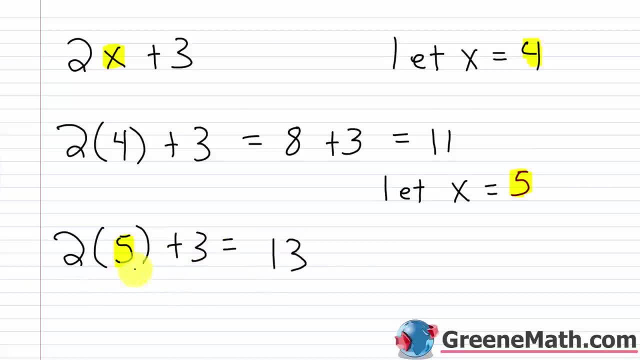 times 5 is 10.. Then 10 plus 3 is 13,. right, And I did that in one step versus 2 up here. Hopefully you can follow. right: 2 times 5 is 10.. Then 10 plus 3 again is 13.. So as I change the, 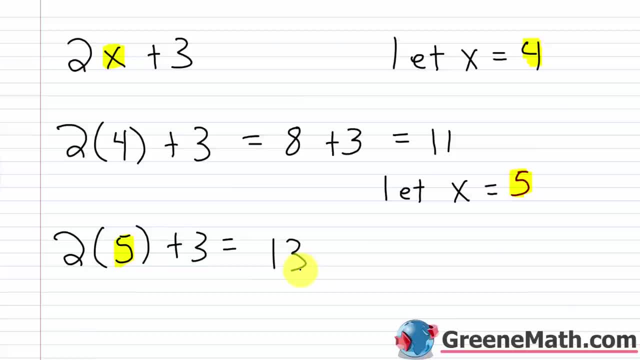 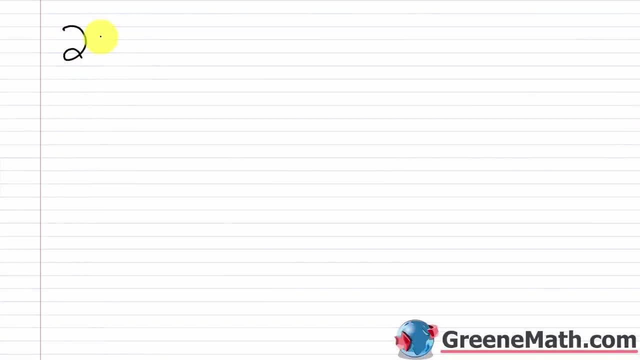 value of x, the value of the algebraic expression will change. Let's do one more. Let's say again 2x plus 3. Let's let x equal negative 2.. So I'm going to plug in a negative 2 for x, right, Very. 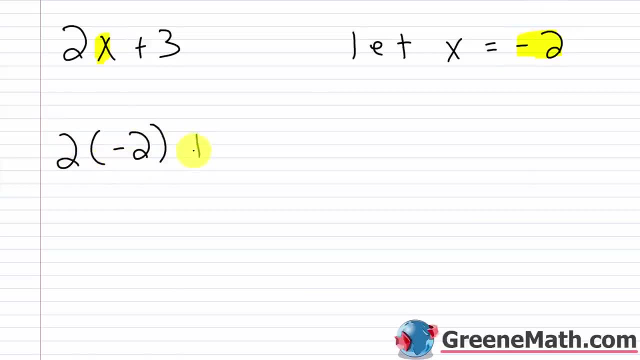 very simple. So 2 times negative, 2 plus 3 equals what, 2 times negative 2.. Remember, positive times, negative is negative. 2 times 2 is 4.. So that's going to give me negative 4,. 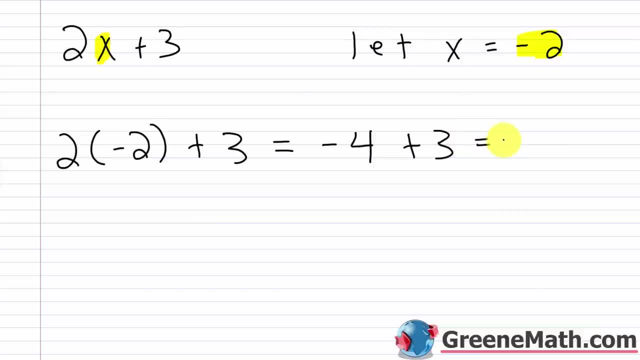 then plus 3.. And at this point we know how to add integers: right: Negative: 4 plus 3 is negative 1. All right, So again, in each case we got a different value for the algebraic expression because we chose a different value for our variable x. So in some cases we can simplify. 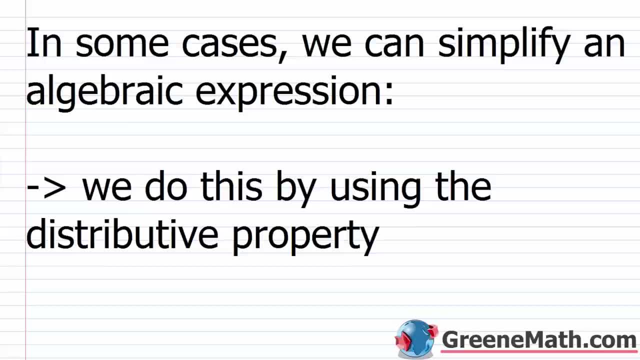 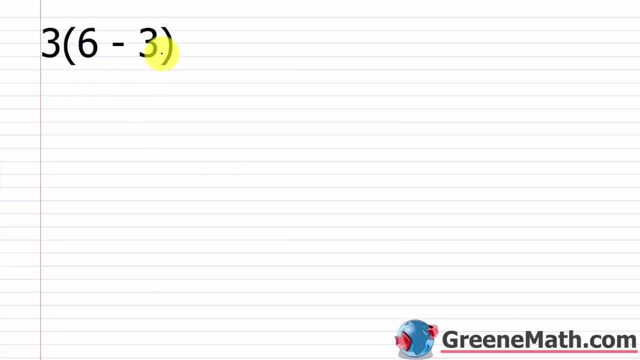 an algebraic expression And we're going to do this using the distributive property. So we learned this back in pre-algebra. And to give you a basic reminder of this, let's say we had something like 3 times this quantity, 6 minus 3.. 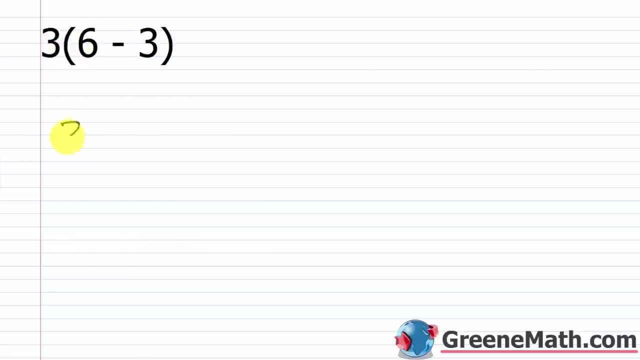 Again, because we have parentheses here. I'm basically saying: what is 3 times the difference of 6 and 3, right? So 6 minus 3 is what That's 3.. So 3 times 3 is 9.. 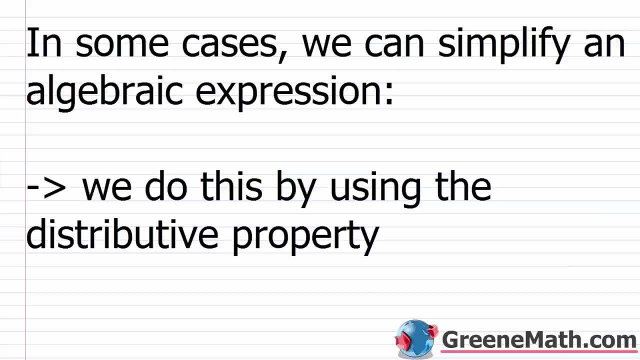 value for our variable x. So in some cases, we can simplify an algebraic expression. And we're going to do this using the distributive property. So we learned this back in pre-algebra. And to give you a basic rule, we're going to use the distributive property. And we're going to use the distributive 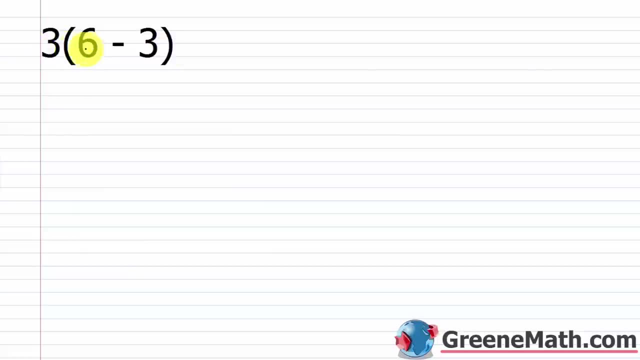 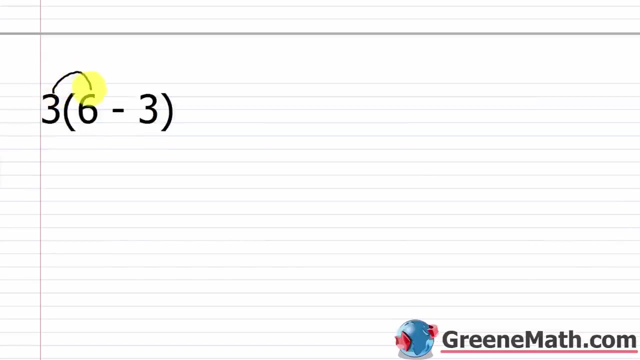 property. So let's say we had something like 3 times this quantity 6 minus 3. Again, because we have parentheses here, I'm basically saying, what is 3 times the difference of 6 and 3, right? So 6 minus 3 is what? That's 3. So 3 times 3 is 9. But we can use the distributive property to do this as well. Remember, because multiplication is distributive over addition or subtraction. So what I can do is I can do this by multiplying by addition or subtraction. So I can do this by multiplying by addition or subtraction. So I can do this by multiplying by addition or subtraction. So I can distribute the 3 to each term inside of the parentheses. Remember, if I have a single number, that's a term, right? A single number, that's a term. So 3 times 6 would give me 18. But let's write it out like this. And then minus, you'd have 3 times 3. 3 times 3. I'll get the same answer as I did before, right? I'm going to get 9 either way. 3 times 6 is 18. And we're subtracting away 3 times 3, which is 9. And 18 minus 9 is 9, right? So either way you do it, you get the same 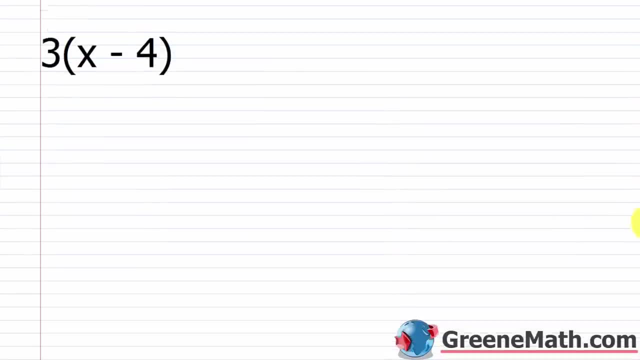 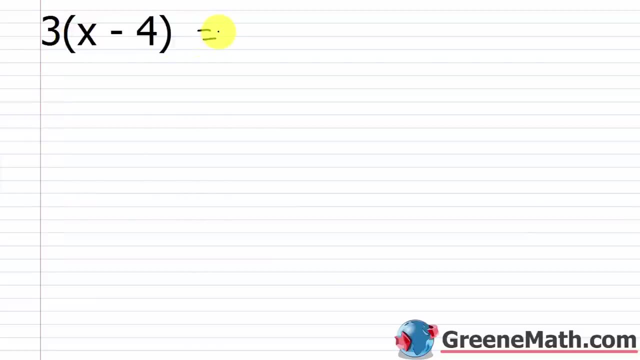 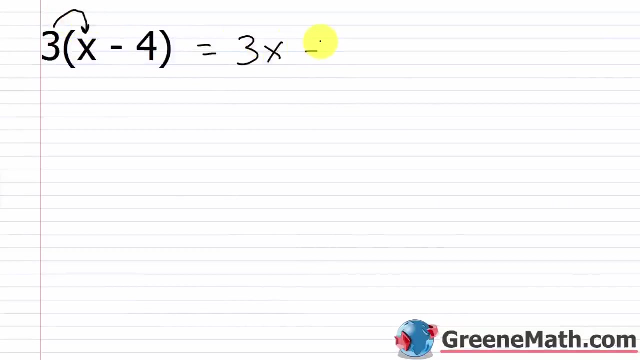 answer. So we're going to use that property here to simplify. We have 3 times this quantity, x minus 4. So what I'm going to do is I'm going to distribute this 3 to each term inside of the parentheses. So 3 times x is 3x. Then minus 3 times 4, which I can write 3 times 4. I can just say 12, right? We know that's 12 at this point. So I've got 3 times 4. I can just say 12. So I've simplified 3 times this quantity, x minus 4, as 3x minus 12. Now, I don't have a single number here as an answer because I still don't know what the value of x is. But I've simplified it a little bit, or some people in some cases are going to want to write it this way. And we'll learn about that later on in Algebra 1, where we're going to reverse what we just did. That's a process called factoring. And again, we're not going to talk about that now. That'll be in a much further lesson. 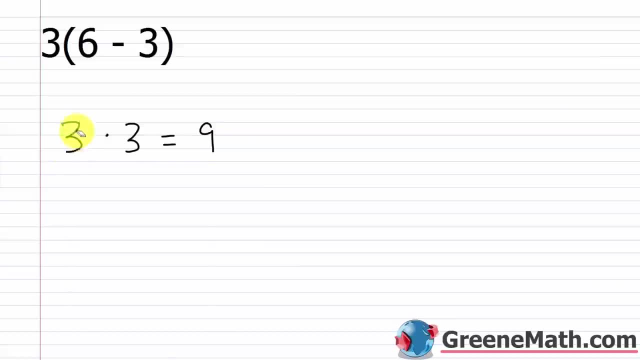 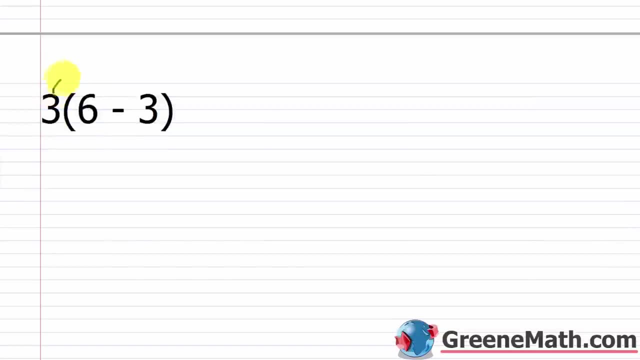 But we can use the distributive property to do this as well, Remember, because multiplication is distributive over addition or subtraction. So what I can do is I can distribute the 3 to each term, inside of the parentheses. Remember, if I have a single number, that's a term, right, A single number, that's a term. 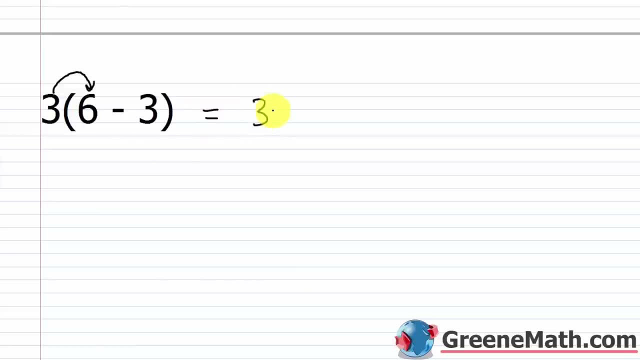 So 3 times 6 would give me 18.. But let's write it out like this: And then, minus, you'd have 3 times 3.. 3 times 3.. I'll get the same answer as I did before. right, I'm going. 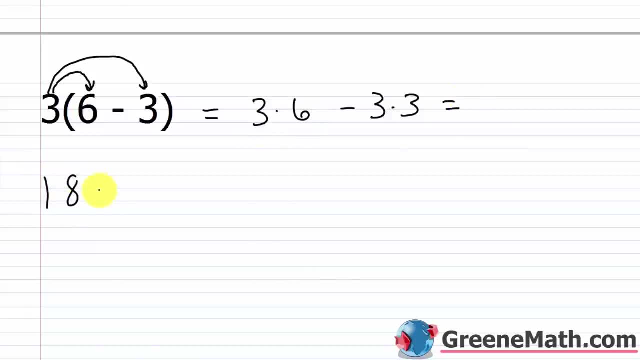 to get 9 either way. 3 times 6 is 18.. And we're subtracting away 3 times 3,, which is 9.. And 18 minus 9 is 9, right? So either way you do it, you get the same answer. 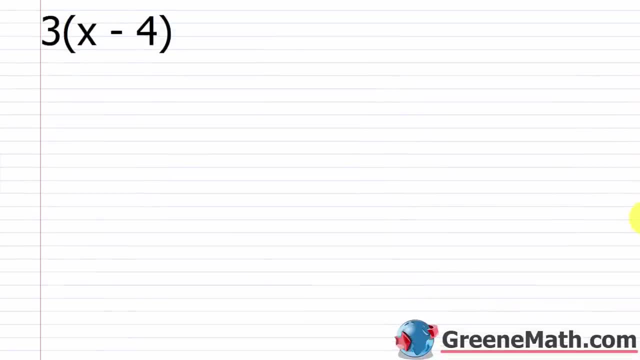 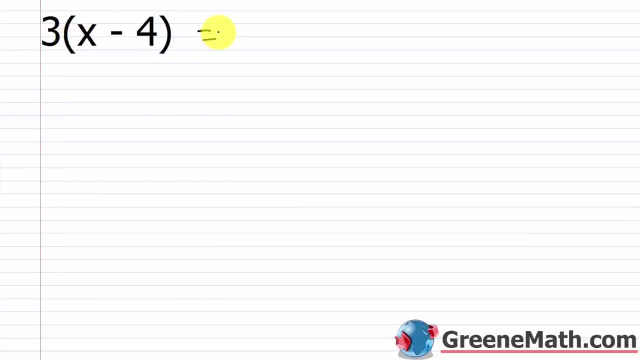 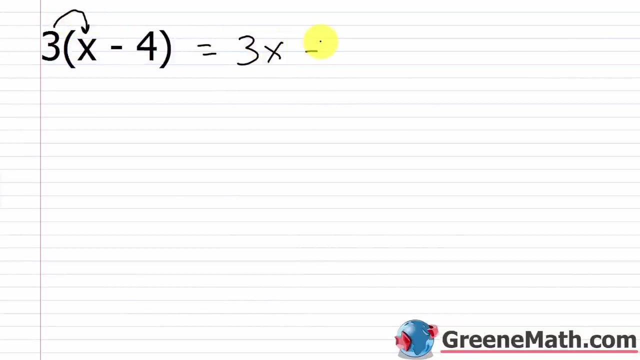 So we're going to use that property here. to simplify, We have 3 times this quantity x minus 4.. So what I'm going to do is I'm going to distribute this 3 to each term inside of the parentheses. So 3 times x is 3x. Then minus 3 times 4,. 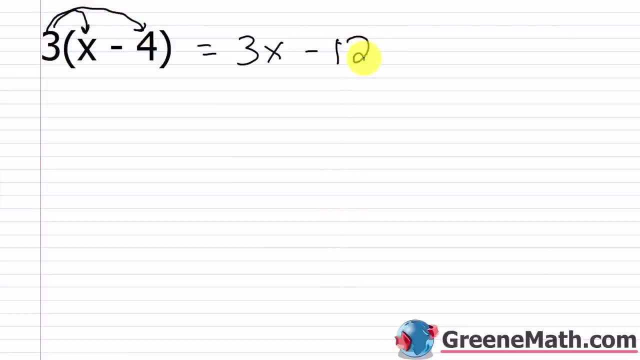 which I can write 3 times 4, I can just say 12, right, We know that's 12 at this point. So I've simplified 3 times this quantity x minus 4, as 3x minus 4.. So I've simplified 3 times this quantity x minus 4, as 3x minus 4.. 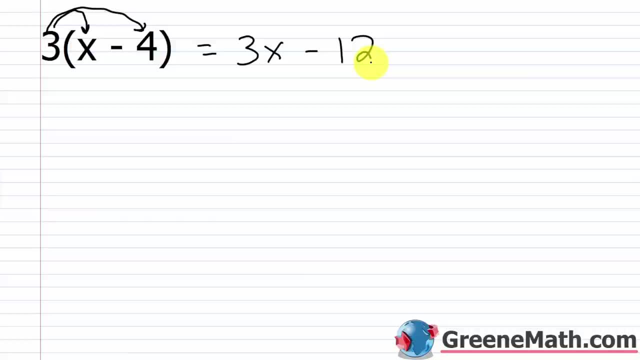 Now I don't have a single number here as an answer, because I still don't know what the value of x is, But I've simplified it a little bit, or some people in some cases are going to want to write it this way, And we'll learn about that later on in Algebra 1, where we're going to. 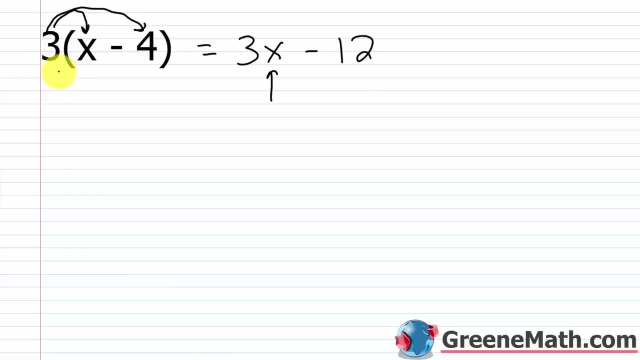 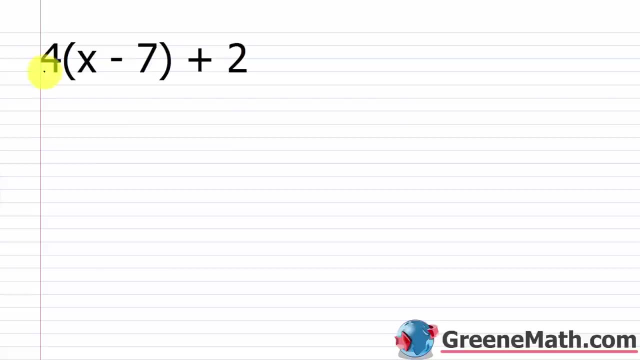 reverse what we just did. That's a process called factoring, And again, we're not going to talk about that now. That'll be in a much further lesson. All right, let's take a look at another one. We have 4 times the quantity x minus 7, plus 2.. So what I'm going to do? 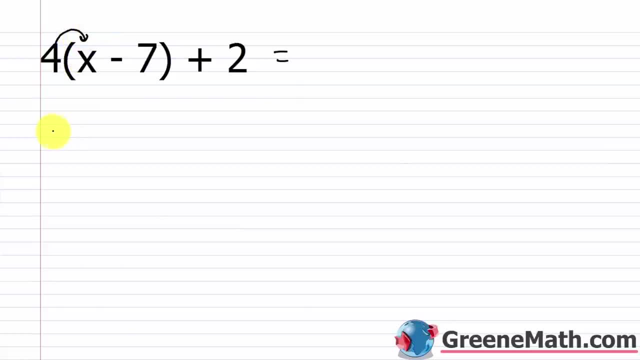 is. I'm going to multiply 4 times x, I'm going to distribute So that'll be 4x, And then we'll have 4 times 7. That's 28. And then plus 2. So at this point I don't know what 4x is right I. 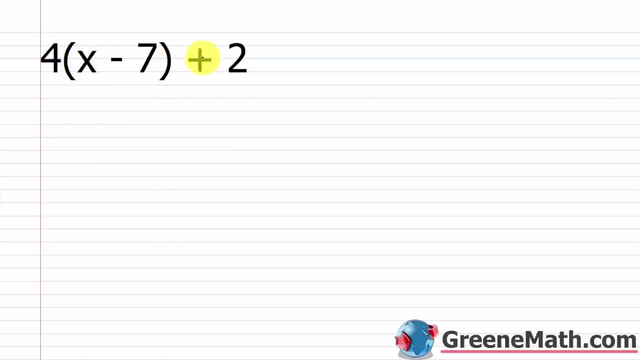 Let's take a look at another one. We have 4 times the quantity x minus 7 plus 2. So what I'm going to do is I'm going to multiply 4 times x. I'm going to distribute. So that'll be 4x. And then we'll have 4 times 7. That's 28. And then plus 2. So at this point, I don't know what 4x is, 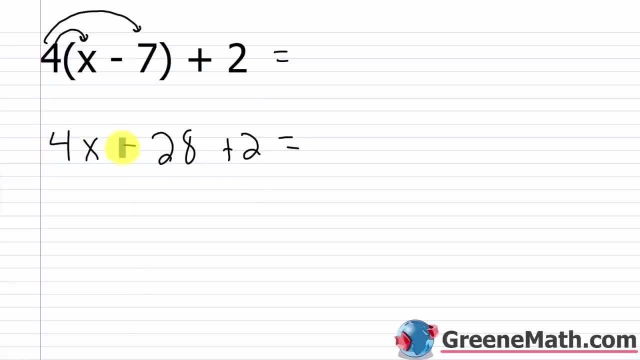 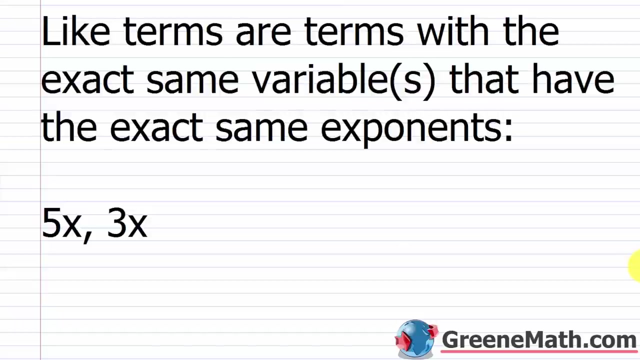 right? I don't have a value of x. But I do know what negative 28 plus 2 is, right? I can do that. And again, if I have minus 28, that's the same thing as negative 28. So that's why I said it that way. So negative 28 plus 2 is going to give me negative 26. So we would have 4x minus 26. All right, now let's talk about like terms. So like terms are 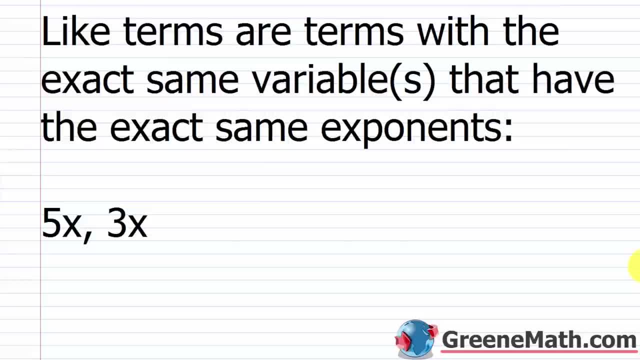 terms with the exact same variable or variables, if there's more than one, that have the exact same exponents. All the variable parts have to be the same. I can't stress that enough. 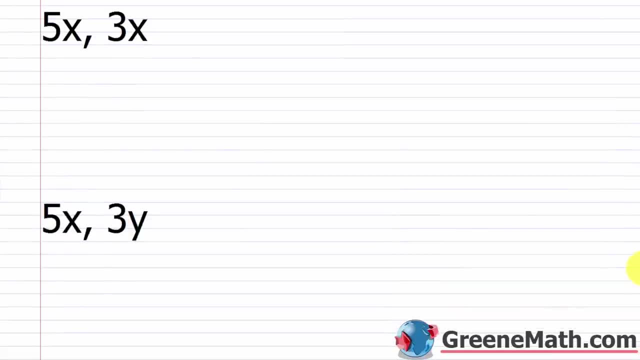 So for example, 5x and 3x are like terms, are like terms. It does not matter what the coefficients are, right? Remember, that's the number that's multiplying the variable or again, variables. It only matters what the variable or variables are. In this case, we have x. In this case, we have x. It's the exact same variable. And so we have like terms. Let's look at 5x and 3y. 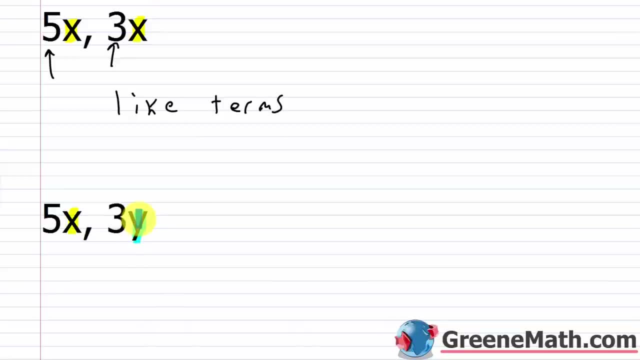 I have x, and then I have y. Those are not the same. Not the same, right? They're different letters. So they're not the same. And so we do not have like terms. These are not like terms. 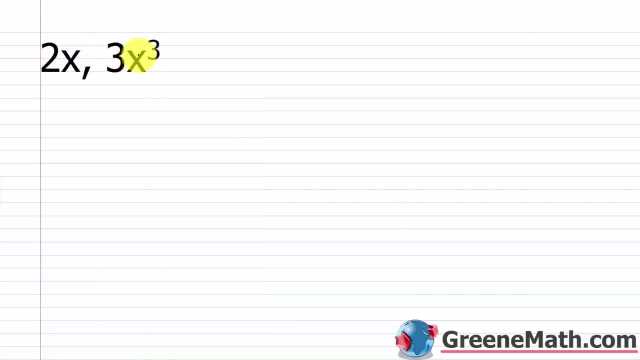 What about 2x and then 3x cubed? Well, they both have the variable of x, but they're not raised to the same power. That's got to be the same. Everything has to be the same. So this stops it from being like terms. So these are not like terms. Not like terms. 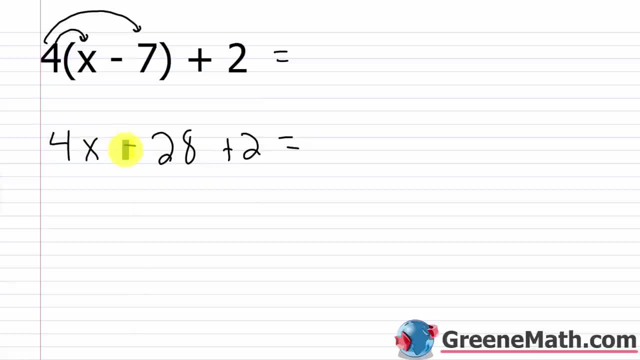 don't have a value of x, But I do know what negative 28 plus 2 is right, I can do that. And again, if I have minus 28, that's the same thing as plus negative 28.. So that's why I said: 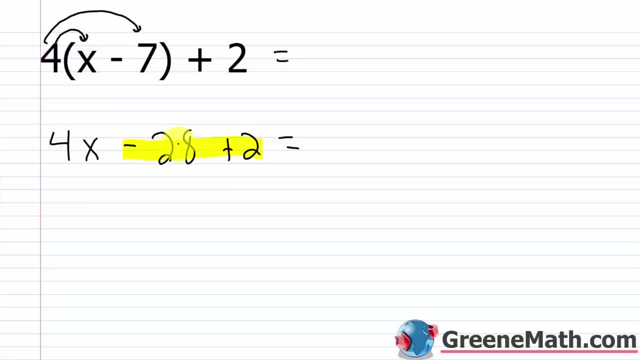 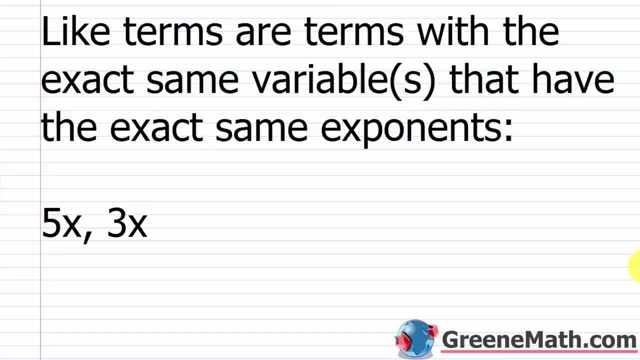 it that way. So negative 28 plus 2 is going to give me negative 26. And then I'm going to multiply 26. So we would have 4x minus 26.. All right, now let's talk about like terms. So like terms are. 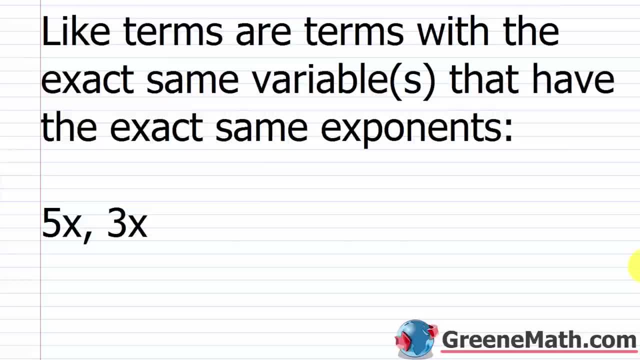 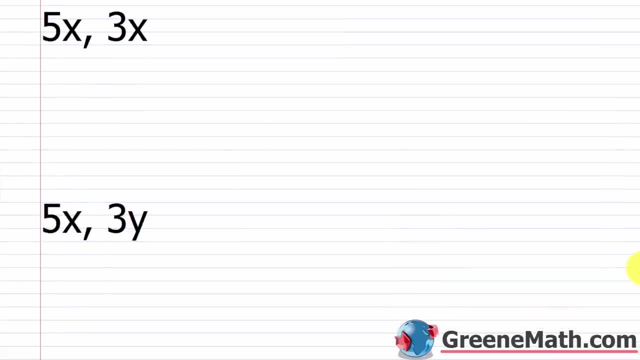 terms with the exact same variable or variables. if there's more than one that have the exact same exponents, All the variable parts have to be the same. I can't stress that enough. So, for example, 5x and 3x are like terms. 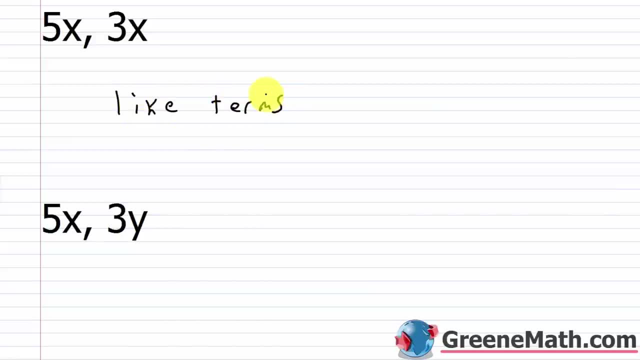 5x and 3x are like terms. It does not matter what the coefficients are, right, Remember? that's the number, that's multiplying the variable, or again, variables. It only matters what the variable or variables are. In this case, we have x. In this case, we have x. It's the exact same. 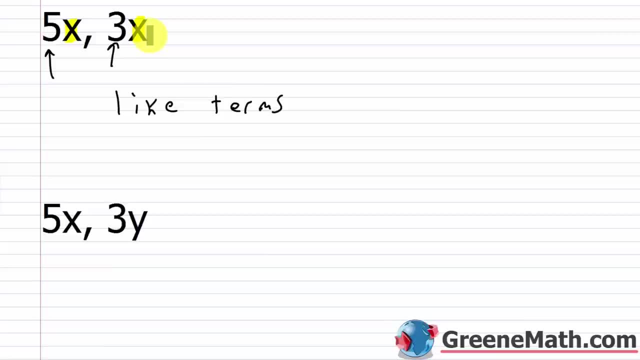 variable, And so we have like terms. Let's look at 5x and 3y. I have x And then I have y. Those are not the same, These are not the same right. They're different letters, So they're not the same, And so we do not. 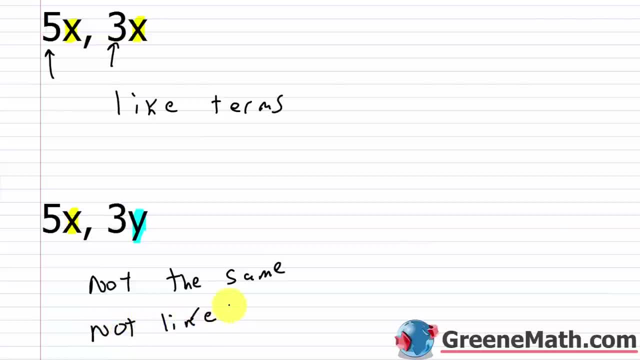 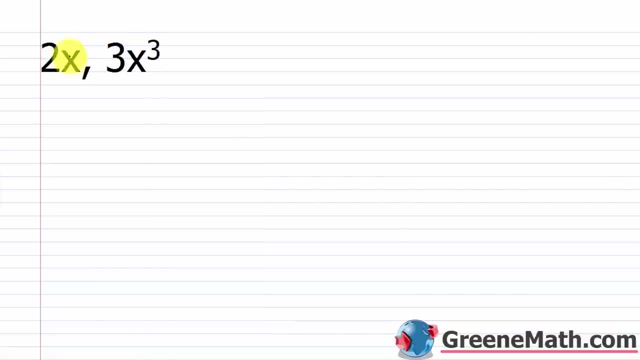 have like terms. These are not like terms. What about 2x and then 3x, cubed? Well, they both have the variable of x, but they're not raised to the same power. That's got to be the same Everything. 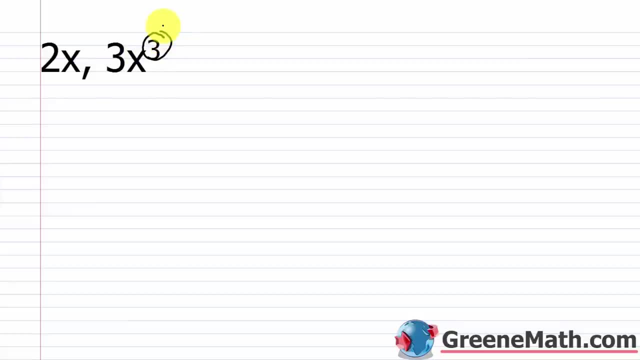 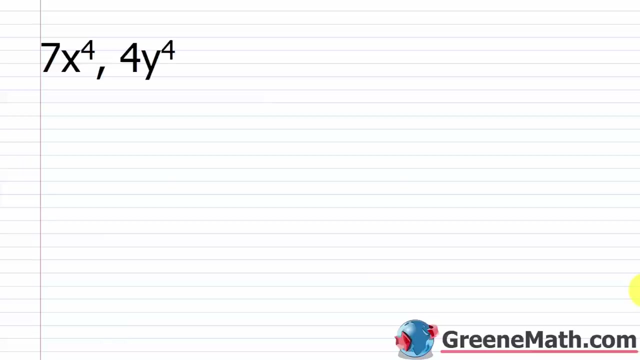 has to be the same. So this stops it from being like terms. So these are not like terms. What about here? We have 7x to the fourth power, 4y to the fourth power. Well, we have the same exponent. Notice how we have each variable raised to the fourth power. But the variable itself is: 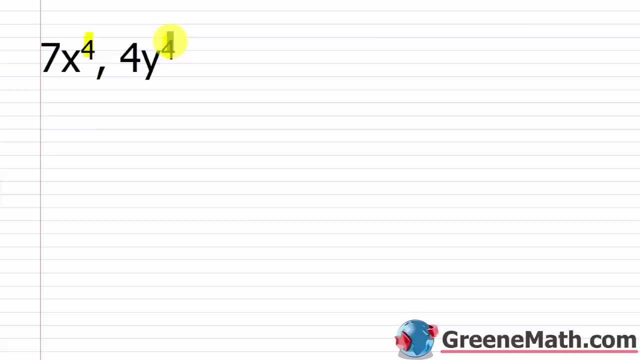 different. One is x, one is y. You can't have anything be different. Again. the coefficients can be different: 7 or 4, or whatever the number parts are. that can be whatever. The variable part has to be the same, And in this case it's not. This is x, This is y, They're. 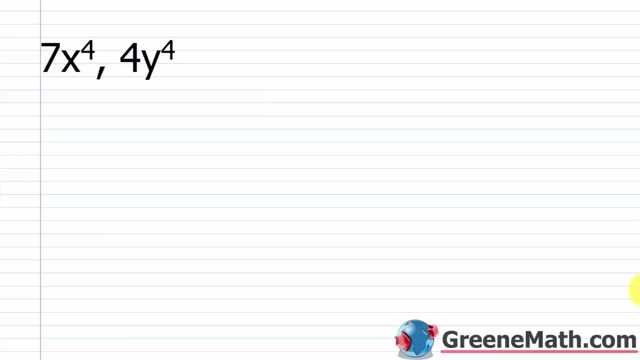 What about here? We have 7x to the fourth power, 4y to the fourth power. Well, we have the same exponent. Notice how we have each variable raised to the fourth power, but the variable itself is different. One is x, one is y. You can't have anything be different. Again, the coefficients can be different. 7 or 4 or whatever the number parts are, that can be 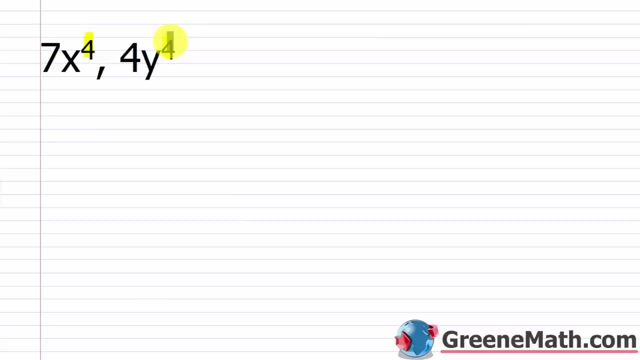 whatever. The variable part has to be the same. And in this case, it's not. This is x, this is y. They're different, and so they're not like terms. 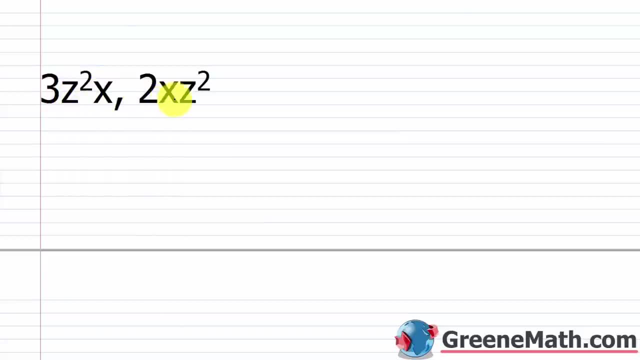 Here we have 3z squared x, and then 2x z squared. So this one might look like they're not like terms. 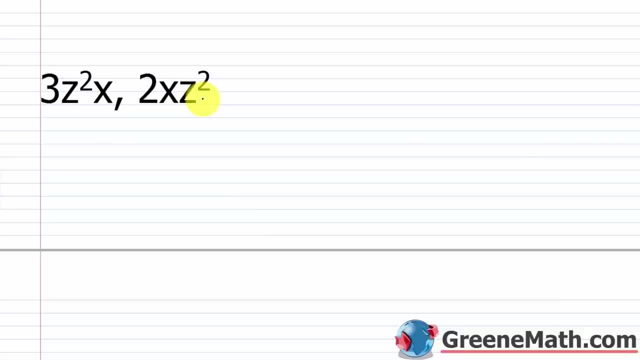 In fact, they are. The variables are presented in a different order. But I want you to remember back from prealgebra that multiplication can occur in any order. That's called the commutative property of multiplication. So if I have 3 times 2, that's the same as 2 times 3. In each case, it's 6. So I can multiply variables in any order. I can have z squared times x, or x times z squared. It doesn't matter. So I have the exact same variables here raised to the same power. I have z squared and z squared. So put a checkmark there. And then I have x and x. Put a checkmark there. And again, the coefficients can be different. So because everything is the same, 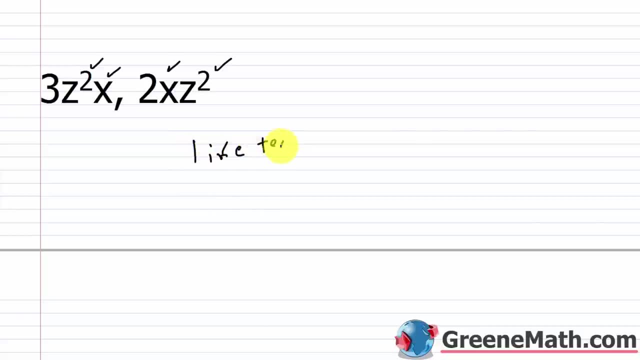 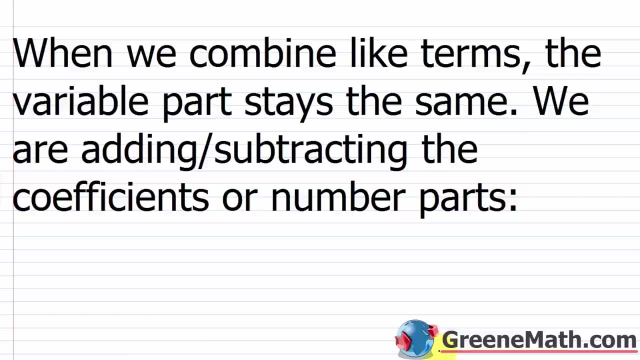 we have like terms. Like terms. Okay, so let's talk a little bit about what we're going to do with these like terms. All right. So when we combine like terms, the variable part stays the same. So if I have x squared and x squared, that doesn't change. 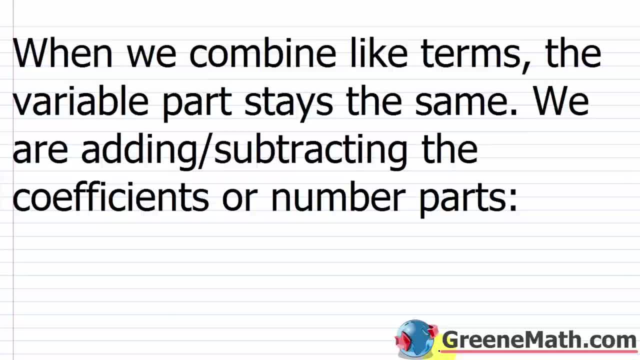 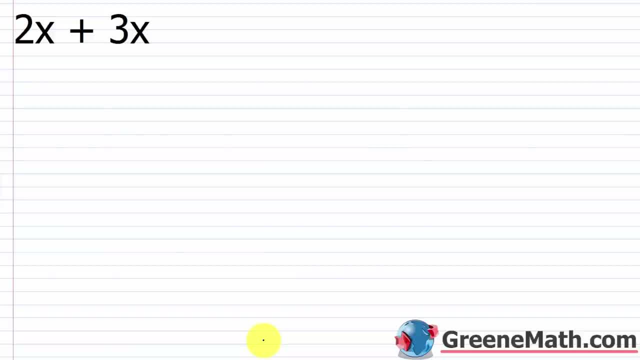 We're just going to be adding and subtracting the coefficients, or again, the number parts. All right. So let's take a look at 2x plus 3x. Nice and easy problem. I want you to imagine if 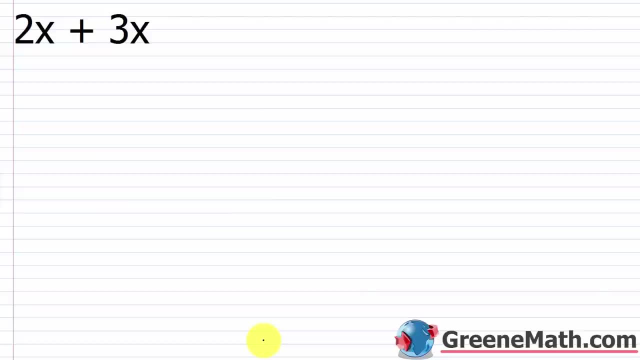 you had two oranges, and you added to that three oranges. Well, everybody knows they'd have five oranges. The easy way to do it is just to leave the variable the same. Just say, okay, I know I'm going to have x. And just add the coefficients. So 2 plus 3 is 5. That's 5x. If you were to visualize what's going on, 2x is x plus x. So x plus 3 is 5x. So 2 plus 3 is 5x. So 2 plus 3 is 5x. 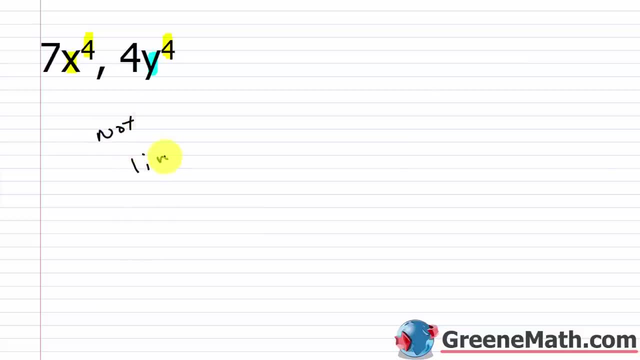 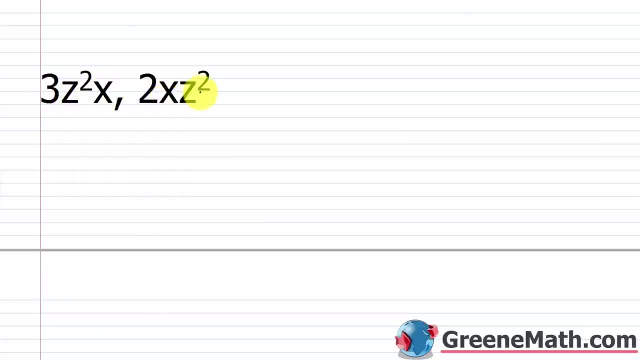 different And so they're not like terms. Here we have 3z squared x and then 2xz squared, So this one might look like they're not like terms, but in fact they are. The variables are presented in a different order, But I want you to remember: if you have a variable that's not like terms, you 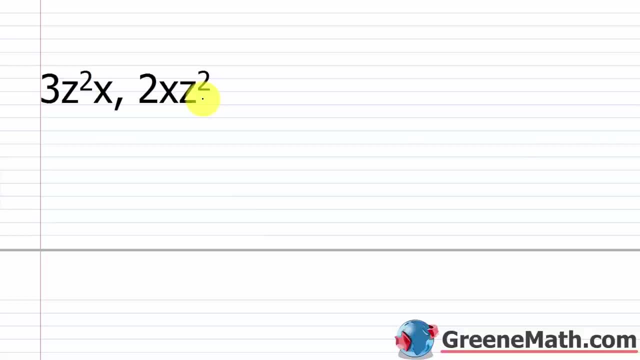 have to remember back from prealgebra that multiplication can occur in any order. That's called the commutative property of multiplication. So if I have 3 times 2, that's the same as 2 times 3.. In each case it's 6.. So I can multiply variables in any order. I can have z squared. 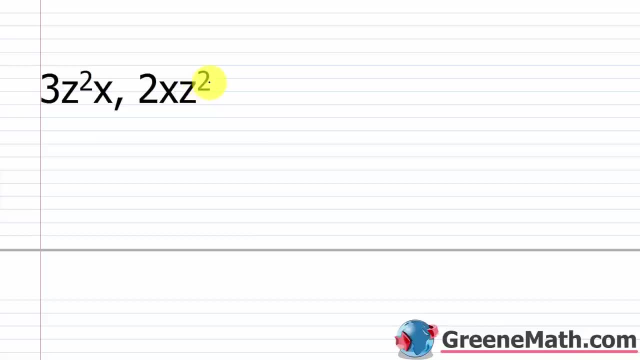 times x or x times z squared, It doesn't matter. So I have the exact same variables here raised to the same power. I have z squared and z squared, So put a checkmark there. And then I have x and x. Put a checkmark there. 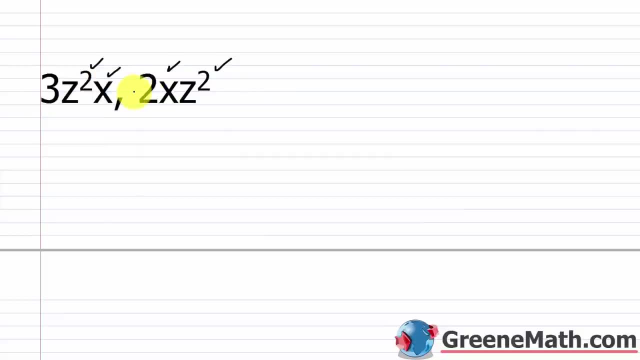 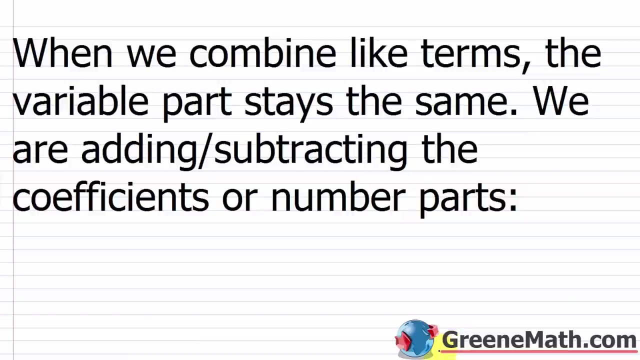 And again, the coefficients can be different. So, because everything is the same, we have like terms, Like terms. Okay, So let's talk a little bit about what we're going to do with these like terms. All right, So when we combine like terms, the variable part stays the same. So, if I have 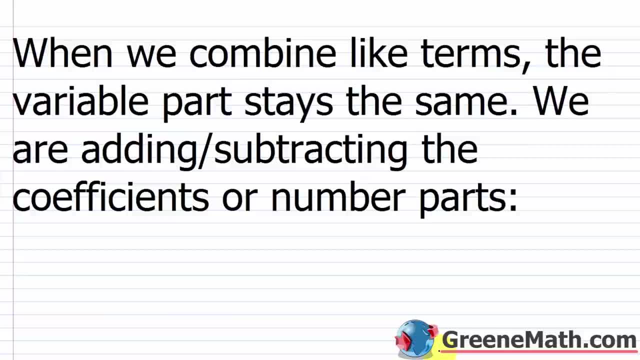 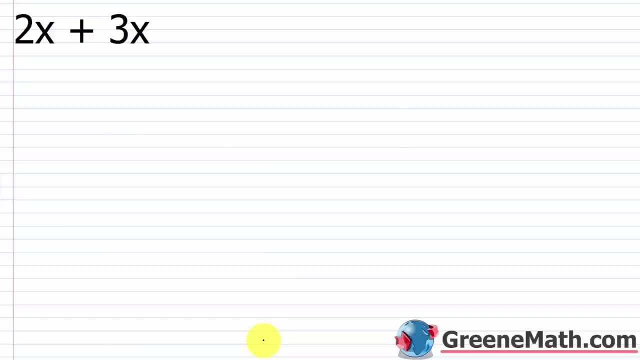 x squared and x squared. that doesn't change. We're just going to be adding and subtracting the coefficients, or again the number parts. All right, So let's take a look at 2x plus the 3x. Nice and easy problem, One should imagine if you had two oranges and you added to that three. 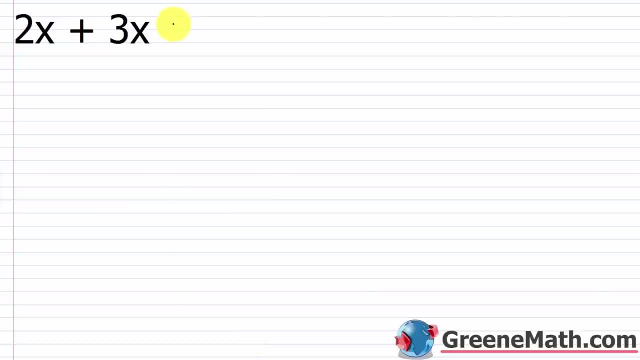 oranges. Well, everybody knows they'd have five oranges. The easy way to do it is just to leave the variable the same, Just say okay, I know I'm going to have x, and just add the coefficients. So 2 plus 3 is 5.. That's 5x. If you were to visualize what's going on, 2x is x plus x, So x plus x. 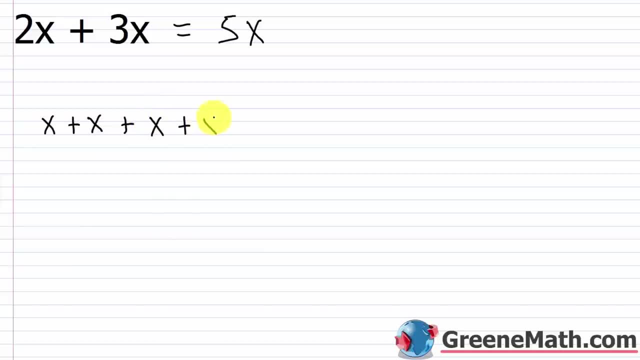 And then 3x is x plus x plus x. If you kind of view it this way, it makes sense. Okay, I have 1,, 2,, 3,, 4,, 5 of these guys, 5x. But 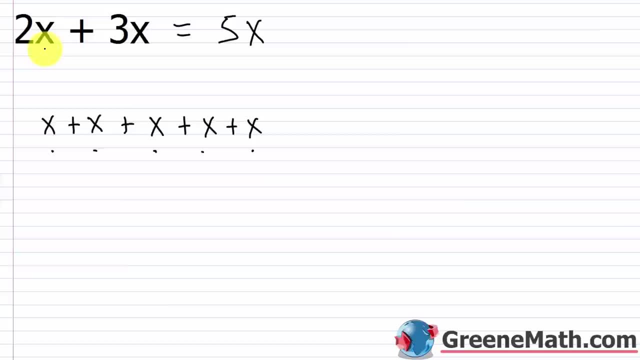 you don't want to do that every time. It's going to slow you down. All right, So you just want to say: okay, the variable part is going to stay the same, So that x is going to stay the same. So I. 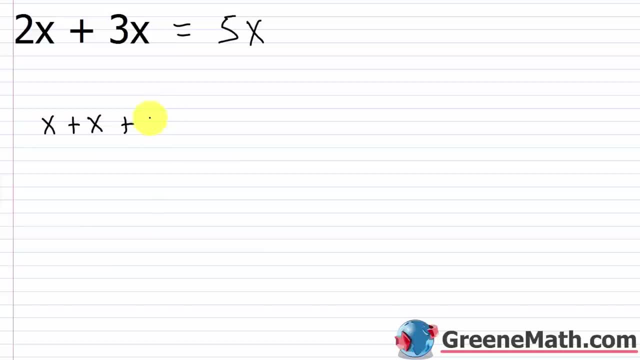 And then 3x is x plus x plus x. And if you kind of view it this way, it makes sense. Okay, I have 1, 2, 3, 4, 5 of these guys, 5x. But you don't want to do that every time. It's going to slow you down. All right. So you just want to say, okay, the variable part is going to stay the same. So that x is going to stay the same. So I just write that first. Then I'm just going to add the coefficient parts. All right. So 2 plus 3 is what? That's 5. So I end up with 5x. And again, if I have something plus 3 of the same thing, I'm going to have 5 of something. So 2 apples plus 3 apples gives me 5 apples. 2 Honda Civics plus 3 Honda Civics gives me 5 Honda Civics, right? So on and so forth. Another way to kind of think about it using the distributive property, and it involves factoring, which we haven't gotten to yet. But if I were to write this for you like this, let's say that I pulled the x out, which is common to both. And I wrote this as x times the quantity 2 plus 3. 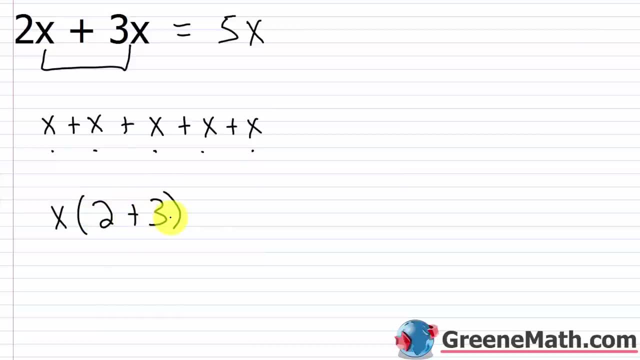 Well, I could do 2 plus 3 first and get 5, multiply 5 times x, end up with 5x. 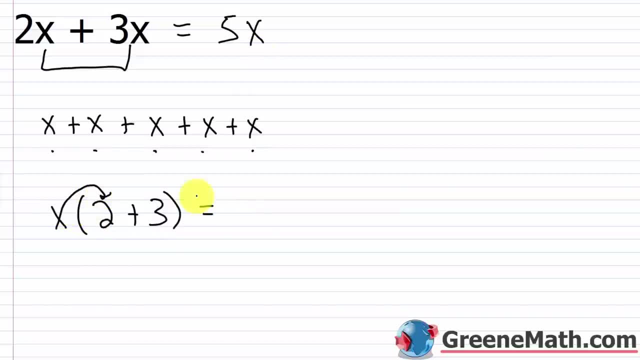 Or I could, again, distribute the x. x times 2 is 2x plus x times 3, which is 3x. And again, you see where we start with this 2x plus 3x. So kind of any way you want to use 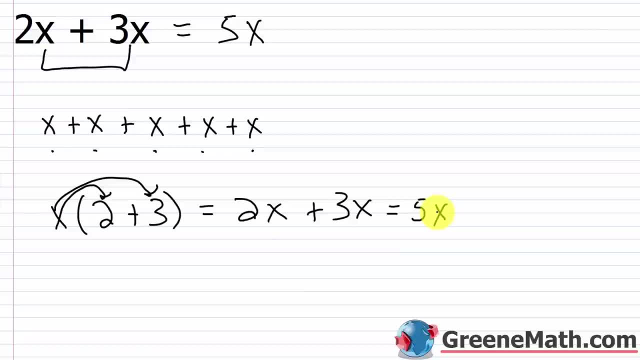 this to visualize what's going on here, it's 2 of something plus 3 of the same thing is giving you 5 of that thing. 2 apples plus 3 apples, 5 apples. 2 oranges plus 3 oranges, 5 oranges. You know, 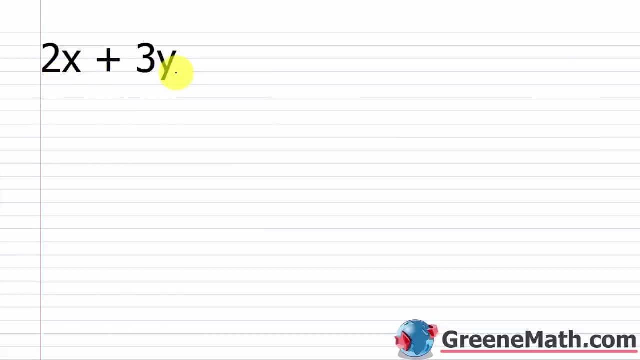 so on and so forth. Here we have 2x plus 3y. Now, we don't have like terms here, so we can't combine them. So let me try to make sense of this for you. If I have 2, let's say, oranges, and I try to add that to 3 apples, well, I still have 2 oranges and 3 apples, right? I can't combine them and say, okay, well, I have 5 orange apples, right? I don't. 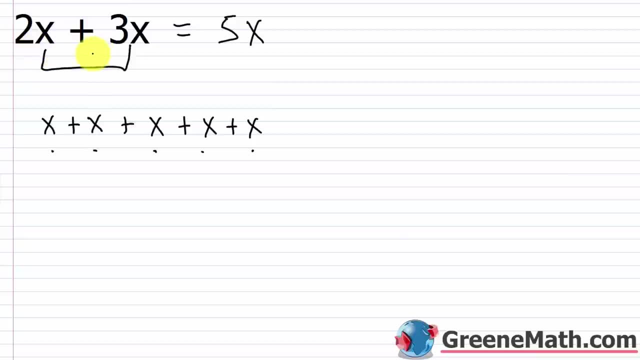 just write that first, Then I'm just going to add the coefficient parts. All right, So 2 plus 3 is what That's, 5.. So I end up with 5x. And again, if I have two of something plus three of the same, 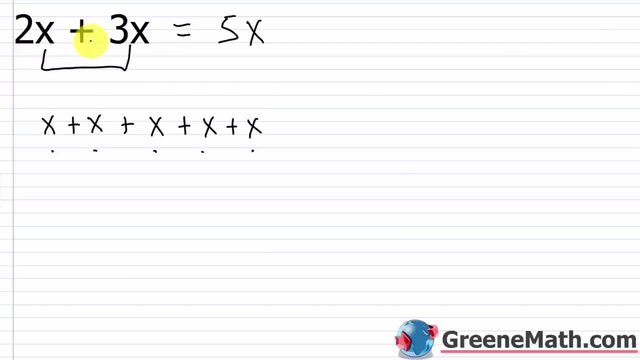 thing I'm going to have five of something. So two apples plus three apples gives me 5x Five apples. Two Honda Civics plus three Honda Civics gives me five Honda Civics. right, So on and so forth. Another way to kind of think about it, using the distributive property, and it involves: 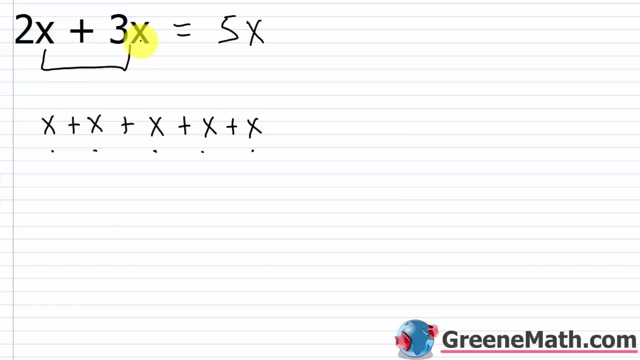 factoring, which we haven't gotten to yet. But if I were to write this for you like this, let's say that I pulled the x out, which is common to both, And I wrote this as x times the quantity 2 plus. 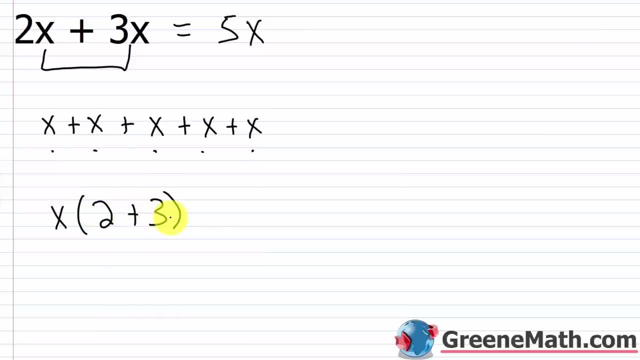 3.. Well, I could do 2 plus 3 first and get 5, multiply 5 times x end up with 5x. Or I could again distribute: the x x times 2 is 2x plus x times 3, which is 3x, And again. 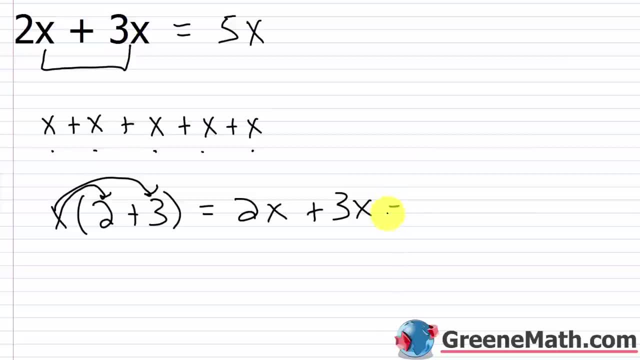 you see where we start with this: 2x plus 3x, So kind of any way you want to use to visualize what's going on here. it's two of something plus three of the same thing is giving you five of that thing: Two apples plus three apples, five apples. Two oranges plus three oranges- five. 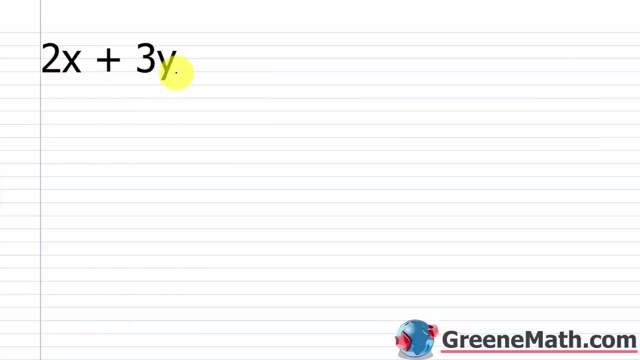 oranges, You know, so on and so forth. So we have 2x plus 3y. Now we don't have like terms here so we can't combine them. So let me try to make sense of this for you. If I have two, let's say, oranges, and I try to add that to three, 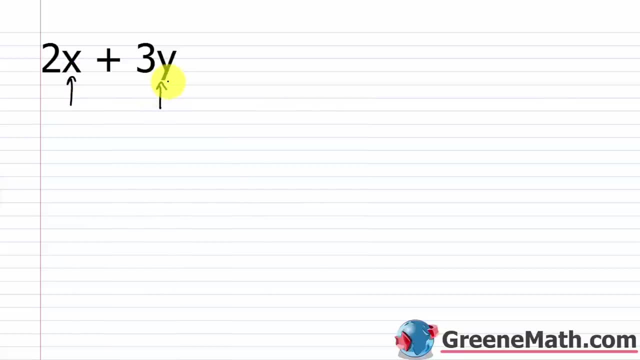 apples. well, I still have two oranges and three apples, right? I can't combine them and say, okay, well, I have five orange apples, right? I don't In the case where we had the same variable, right? 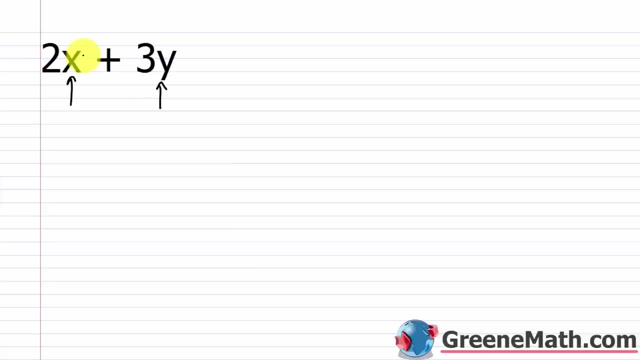 we had like terms. well, yeah, I'm adding the same thing. So if I have again two oranges plus three oranges, right, I can't combine them. So I can't combine them, So I can't combine them, So I can't. 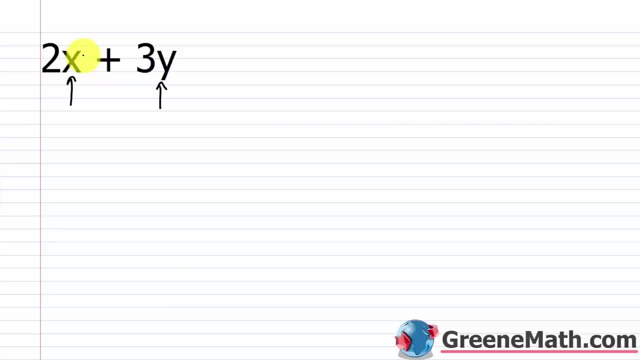 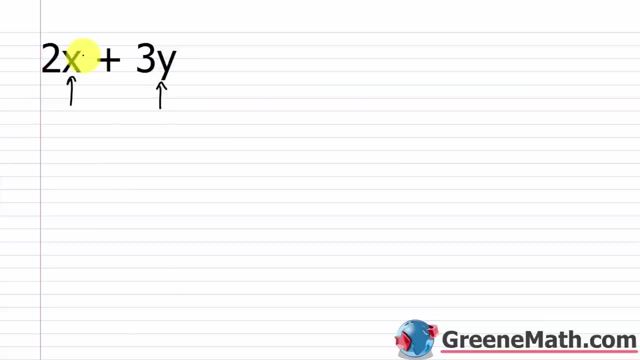 In the case where we had the same variable, right, we had like terms, yeah, I'm adding the same thing. So if I have, again, 2 oranges plus 3 oranges, I have 5 oranges. If I have 2 apples plus 3 apples, I have 5 apples. But if I have 2 oranges plus 3 apples, I just have 2 oranges and 3 apples. So there's no way to kind of, you know, combine these. It's still going to just be 2x plus 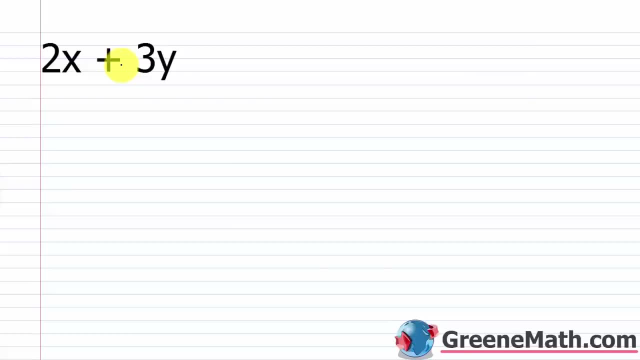 3 oranges. So if you don't have like terms, you really can't simplify, right, in this scenario. 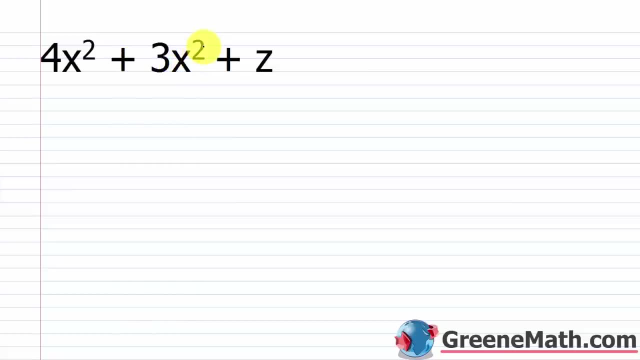 All right, here we have 4x squared plus 3x squared plus z. Now, look for your like terms. I have x squared and x squared. So these two are like terms. These are like terms, and so we can combine them. And I missed an r there. The z is not common to anything, right? So we're not gonna have terms with just the z. So what you do in this scenario is you just combine what you can. 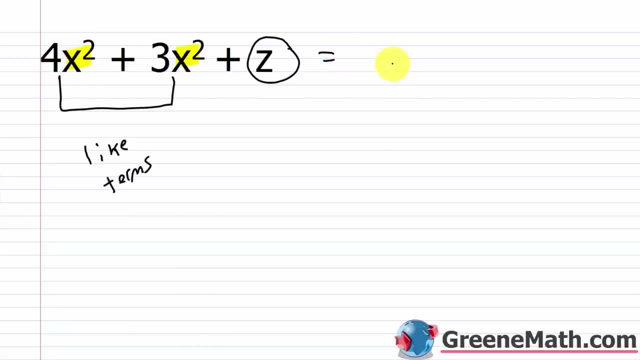 So 4x squared plus 3x squared, again, leave the variable part the same. So leave that x squared part the same, and then just add your coefficients. So what is 4 plus 3? That's 7. So I have 7x squared, and then just copy the rest, so plus c. So when we simplify this algebraic expression, we end up with 7x squared plus c, right? Again, you combine what you can, right? In this case, 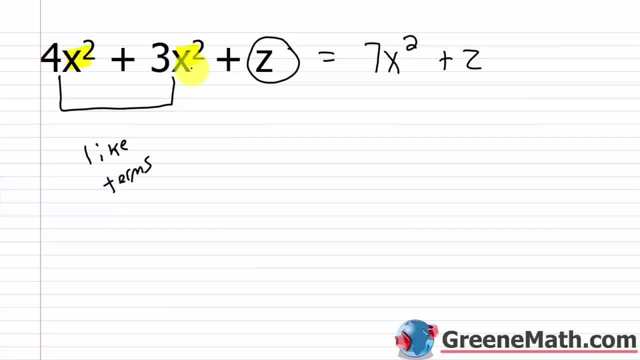 we could combine the like terms 4x squared and 3x squared. All right, here's one that's a little bit more challenging. We have negative 2 times the quantity 4x minus 7 plus 4 times the quantity 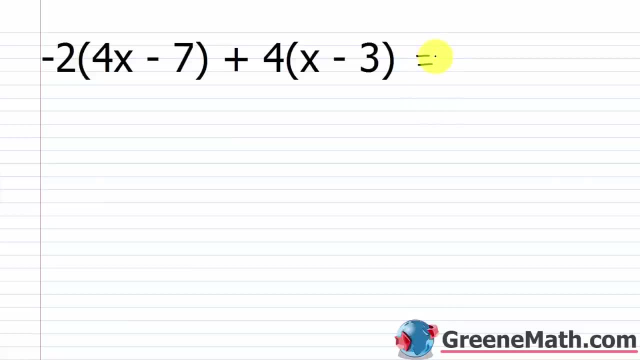 x minus 3. So the first thing I'm going to use is the distributive property to kind of simplify this a bit. So I'm going to multiply negative 2 times 4x, and that's going to give me negative 8x squared. So I'm going to multiply negative 2 times 4x, and that's going to give me negative 8x, and then I'm subtracting away negative 2 times 7, which is going to be negative 14. Now, I'd end up with minus and negative 14, which is the same as plus 14. Now, plus, I'm going to do the same thing over here. We have 4 times x, that's 4x, and then minus 4 times 3, that's 12. 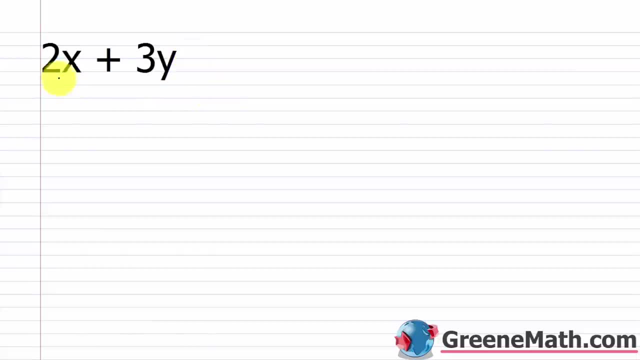 have two oranges and three apples. So there's no way to kind of, you know, combine these. It's still going to just be 2x plus 3y. So if you don't have like terms you really can't simplify. 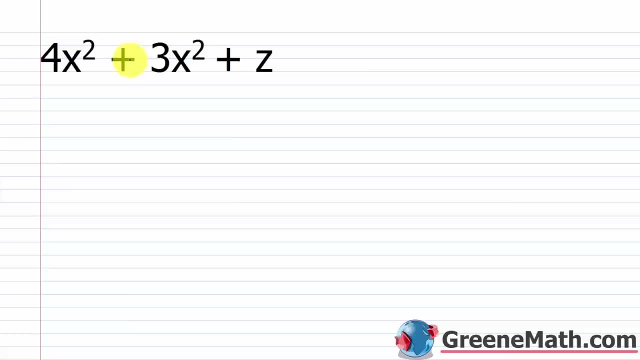 right in this scenario? All right, here we have 4x squared plus 3x squared plus z. Now look for your like terms. I have x squared and x squared, So these two are like terms, These are like terms. 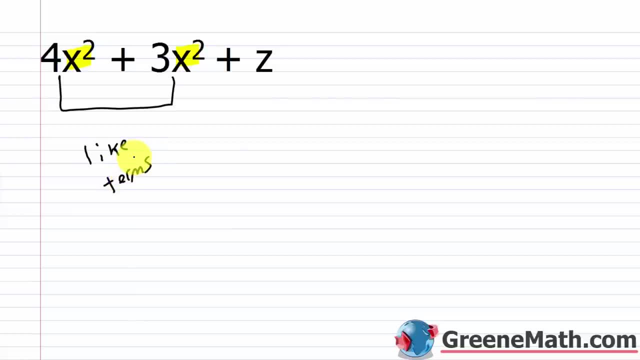 And so we can combine them. And I missed an r there. The z is not common to anything right, So we're not going to have like terms with just the z. So what you do in this scenario is you just combine what you can. 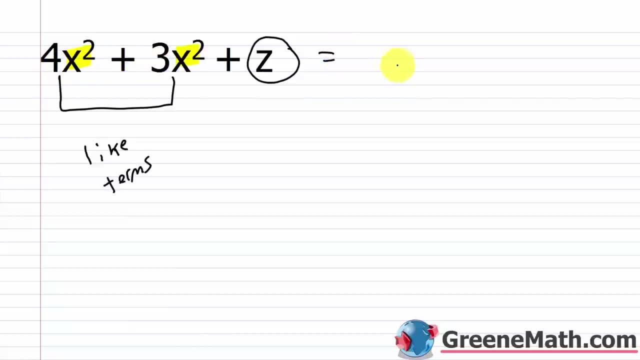 So 4x squared plus 3x squared Again, leave the variable part the same. So leave that x squared part the same, And then just add your coefficients. So what is 4 plus 3?? That's 7.. So I have 7x squared. 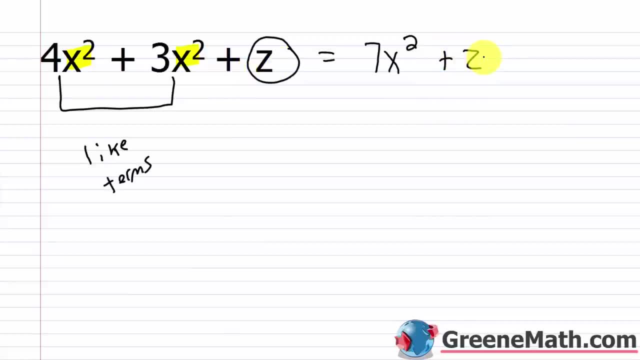 And then just copy the rest: So plus c. So when we simplify this algebraic expression, we end up with 7x squared plus c. right Again, you combine what you can right? In this case we could combine the like terms 4x squared and 3x squared. 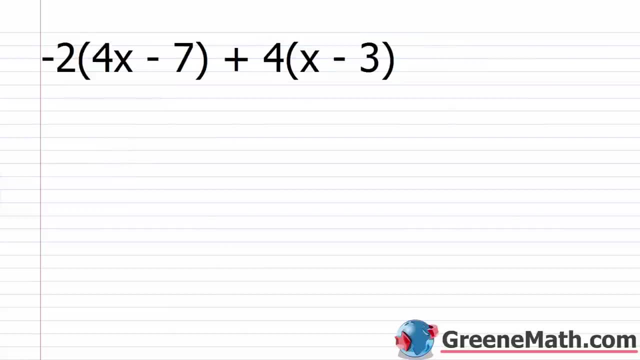 All right, here's one that's a little bit more challenging. We have negative 2 times the quantity 4x minus 7, plus 4 times the quantity x minus 3.. So the first thing I'm going to use is the distributive property to kind of simplify this a bit. 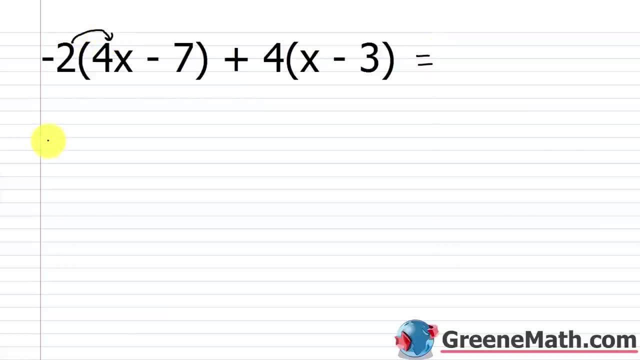 So I'm going to multiply negative 2 times 4x, and that's going to give me negative 8x. And then I'm subtracting away negative 2 times 7,, which is going to be negative 14.. Now I'd end up with minus and negative 14,, which is the same as plus 14.. 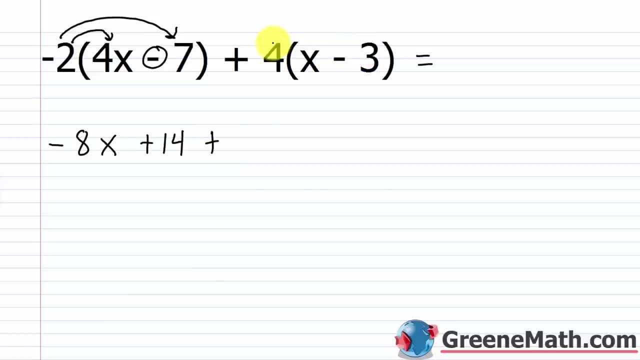 Now plus- I'm going to do the same thing over here. We have 4 times x, That's 4x. And then minus 4 times 3. That's 12.. And so now we're going to look for like terms. 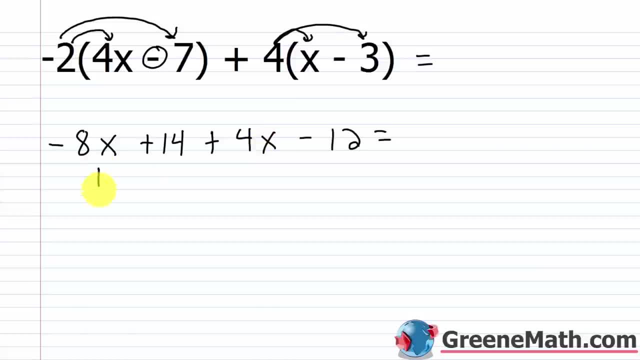 So I have negative 8x and 4x. Those are like terms. right, The variable is x. right, There's no power. You can think of the power as being 1, right, So in each case you have the same thing. 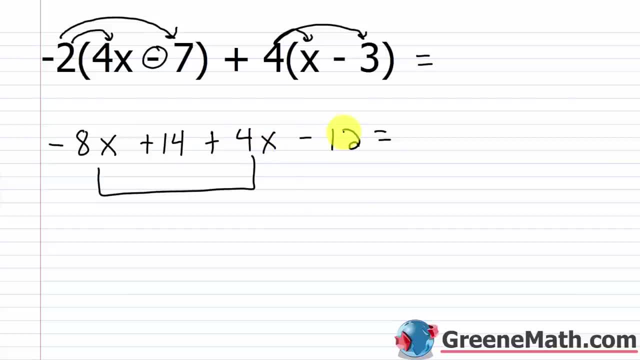 And then you have 14 and negative 12. Those are just numbers or constants. Those can be combined. So let's start out with just Just negative 8x plus 4x. Well, the variable is going to stay the same. 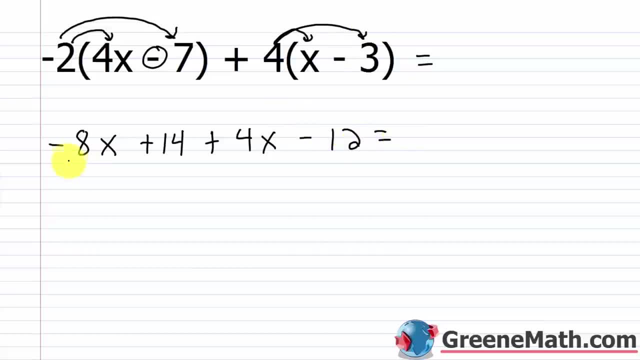 And so now we're going to look for like terms. So I have negative 8x and 4x, those are like terms, right? The variable is x, right? There's no power. You can think of the power as being 1, right? So in each case, you have the same thing. And then you have 14 and negative 12. Those are just numbers or constants. Those can be combined. So let's start out with just negative 8x plus 4x. Well, the variable is going to stay the same. So that's just going to be x. And then think about the coefficients. So what is negative 8 plus 4? Well, negative 8 plus 4 is going to give me negative 4. So this is going to be negative 4x. And then I'm just going to combine the number parts. So I have 14 minus 12. That's going to give me 2, so plus 2. So the answer here would be negative 4x plus 2. And I can't simplify this any further because I don't 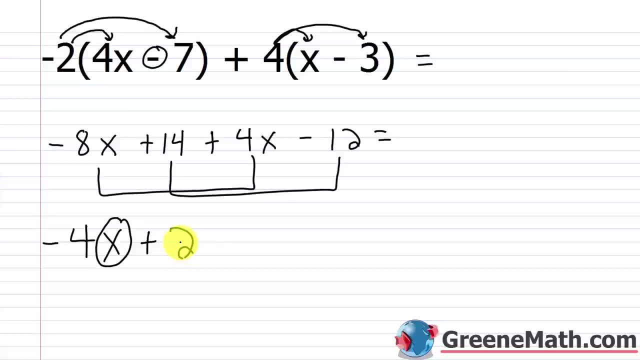 know what the value of x is. So I can't combine this with 2, right? I can't really simplify this unless you give me a value for x. If you said, hey, let x equal this, then I could give you a value for the algebraic expression. But without the value of x, I can't simplify this. So I can't simplify this. So without that, I'm kind of stuck here. Hello, and welcome to Algebra 1, 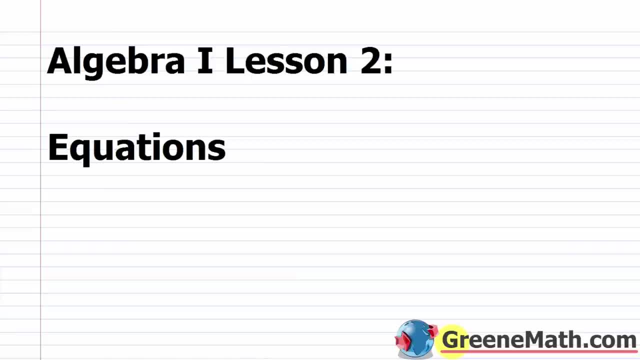 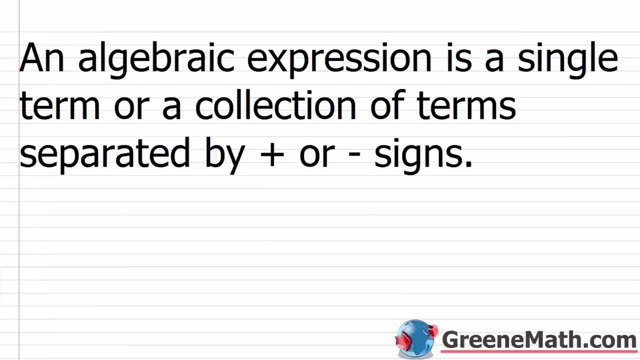 Lesson 2. In this video, we're going to learn about equations. So in our last lesson, we learned a lot of definitions that were going to help us out throughout our study of algebra. Two of those 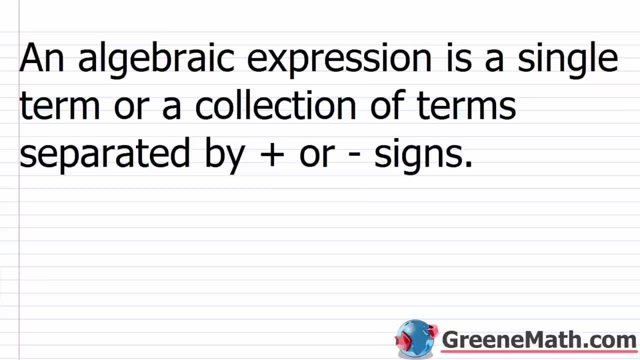 definitions that we're going to review here, one would be that of a term, right? A term is a single number or a number that is multiplied by one or many variables. And those variables can be two powers. Now, we also have something known as an algebraic expression. And an algebraic expression is a single term, right? So it could just be one term, or a collection of terms separated by plus 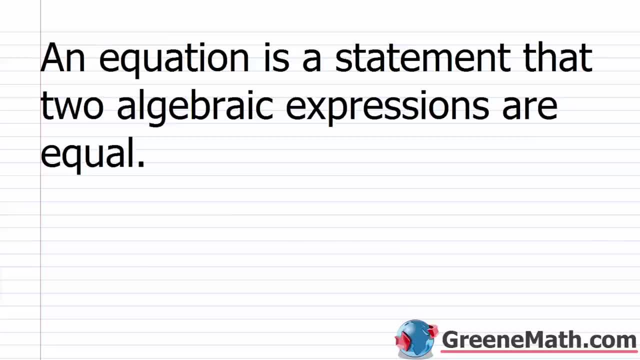 or minus signs. All right, now let's move on and talk a little bit about equations. So an equation is a statement that two algebraic expressions are equal. All right, so this next point is going to be very, very important. And it's going to be a statement that two algebraic expressions are equal. 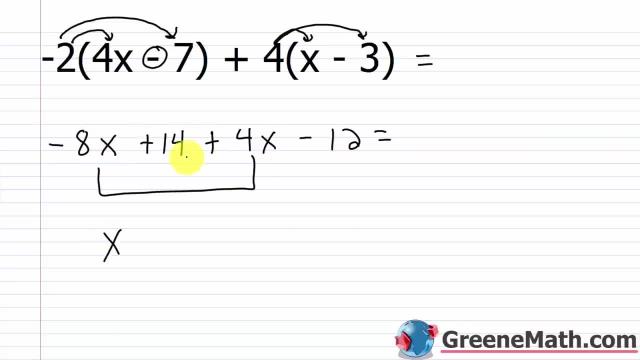 So that's just going to be x. And then think about the coefficient. So what is negative 8 plus 4?? Well, negative 8 plus 4 is going to give me negative 4.. So this is going to be negative 4x. 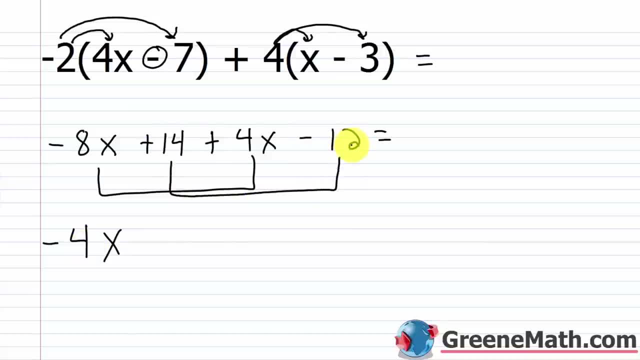 And then I'm just going to combine the number parts, So I have 14 minus 12.. That's going to give me 2.. So plus 2.. So the answer here will be negative: 4x plus 2.. And I can't simplify this any further because I don't know what the value is. 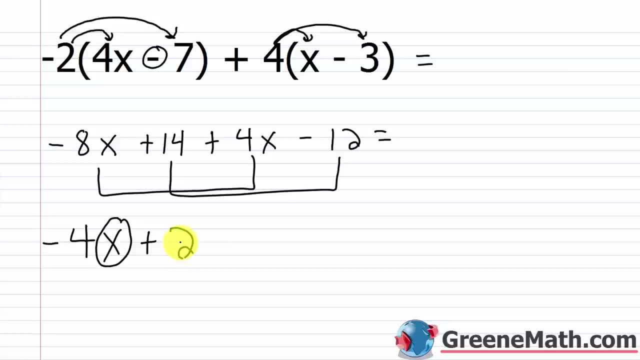 So I can't combine this with 2, right? I can't really simplify this, unless you give me a value for x. If you said, hey, let x equal this, then I could give you a value for the algebraic expression. 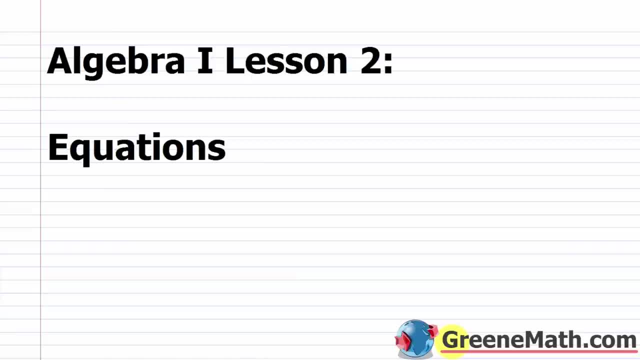 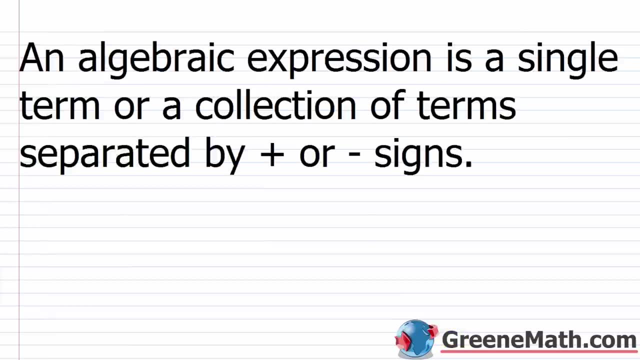 But without that I'm kind of stuck here. Hello and welcome to Algebra 1, Lesson 2.. In this video we're going to learn about equations, So in our last lesson we learned a lot of definitions that were going to help us out. 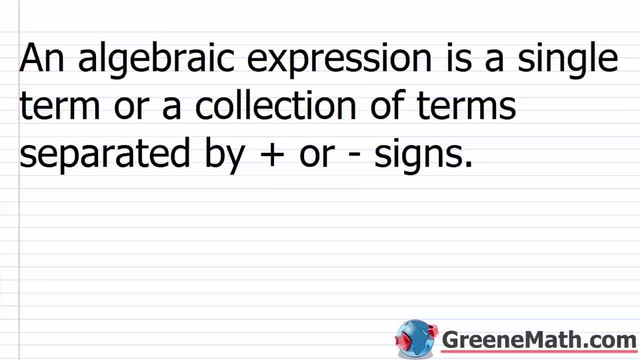 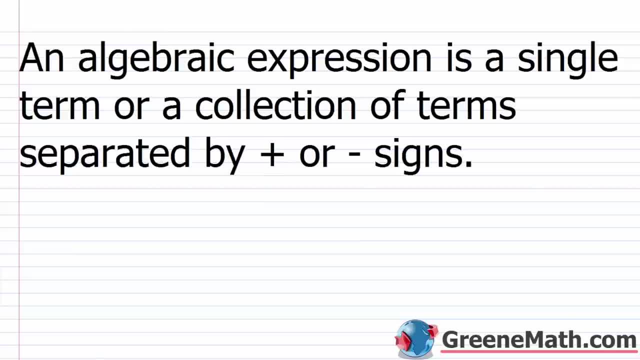 So in our last lesson we learned a lot of definitions that were going to help us out throughout our study of algebra. is a single number, or a number that is multiplied by one or many variables, and those variables can be raised to powers. Now we also have something known as an 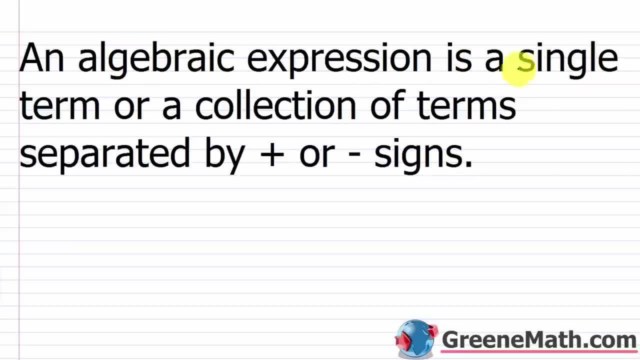 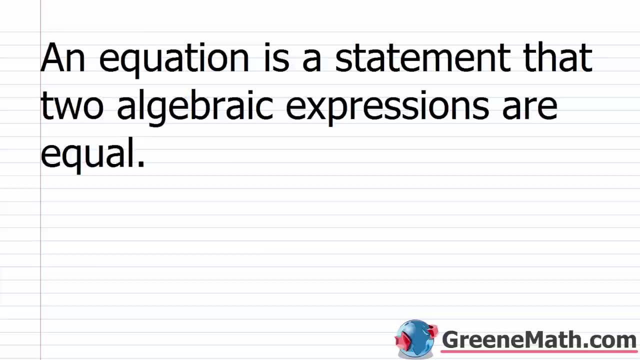 algebraic expression. and an algebraic expression is a single term, right? so it could just be one term or a collection of terms separated by plus or minus signs. Alright, now let's move on and talk a little bit about equations. So an equation is a statement that two algebraic expressions are equal. Alright, 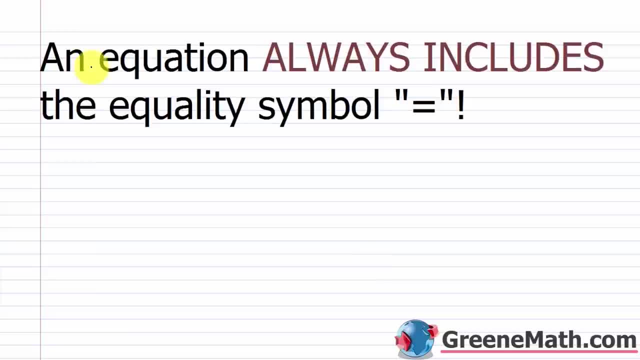 so this next point is going to be very, very important. An equation always includes the equality symbol. So always includes the equality symbol. So when you've looked at the algebraic expressions, we only put an equal symbol in once we get to the end of the equation. So when you've looked at the algebraic expressions, we only put an equal symbol in once we get. 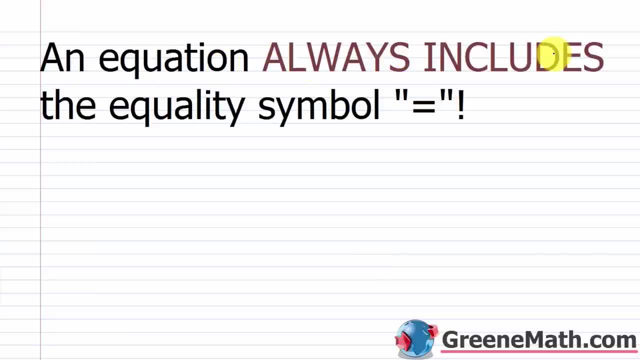 An equation always includes the equality symbol. So always includes the equality symbol. So when you've looked at the algebraic expressions, we only put an equal symbol in once we get a value for it, right? So as an example, let's say I had something like 3x minus 4. This is an algebraic expression. This is an algebraic expression. 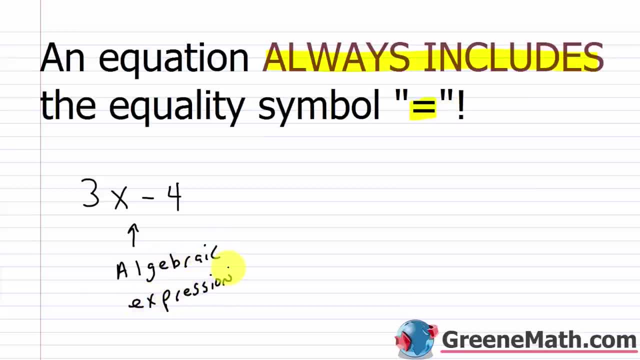 Now, I can't really do anything with this. When I have an algebraic expression, I can simplify it, or I can plug in for the variable if you give me a value. So if I said let x equal 2, I could plug a 2 in there, and I could evaluate, right? And in that particular case, you might see an equal sign because I'm saying, hey, if x equals 2, this algebraic expression is equal to this value. So I can plug in for the variable if you give me a value. So if I said, 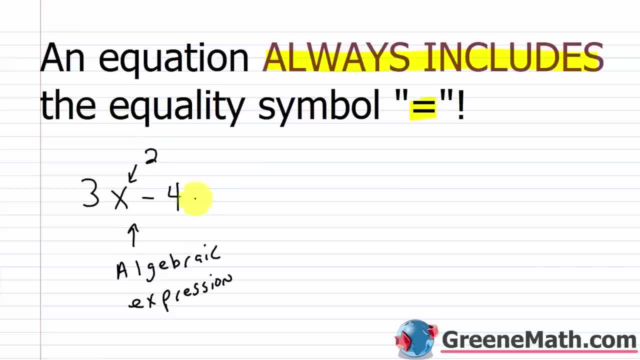 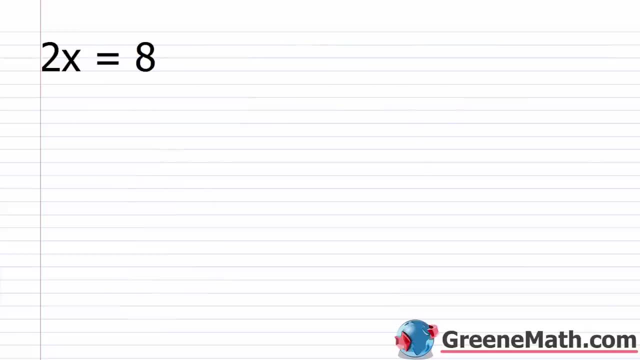 right, but it didn't start out with an equal sign, right? There's nothing there other than 3x minus 4 at this point. So that's an algebraic expression. An equation is going to look like 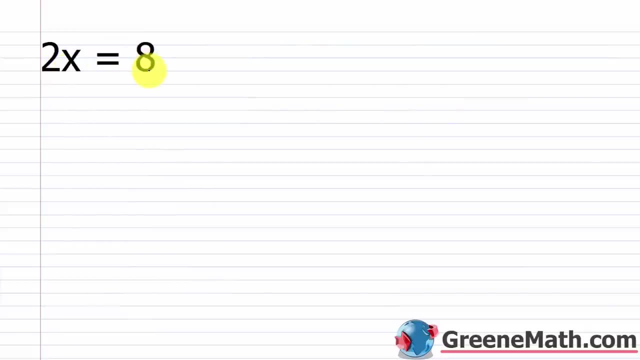 this. We have 2x is equal to 8. So that's the main difference. If you're just starting out in algebra, and you get a test, and you see 2x equals 8, well, okay, it has an equal sign to start. So this is an equation. This is an equation. That's your number one, way to tell, right? It's got an equal sign. It's an equation. You see something like 7x squared minus 1. Okay, no equal sign. This is an algebraic expression. 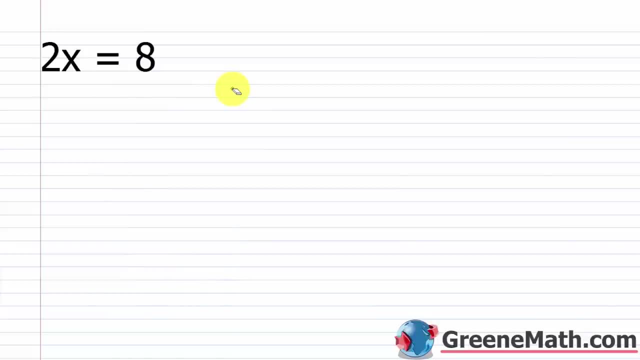 So let's talk a little bit about equations now. And we're not going to get to solving equations until the next lesson. We're just going to learn some of the basics of equations now so that we can just kind of lightly introduce. 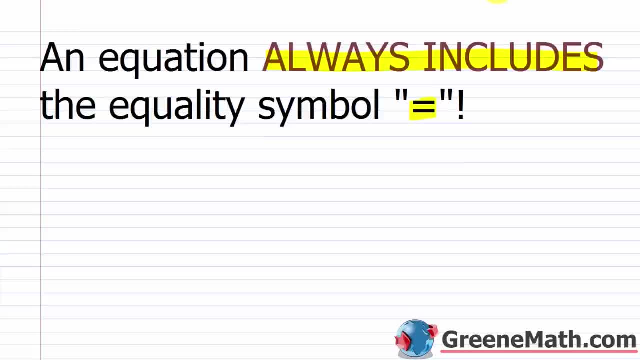 a value for it. Alright, so as an example, let's say I had something like 3x minus 4.. This is an algebraic expression. A man for it who doesn't. this is an algebraic expression, A man for it who has a. 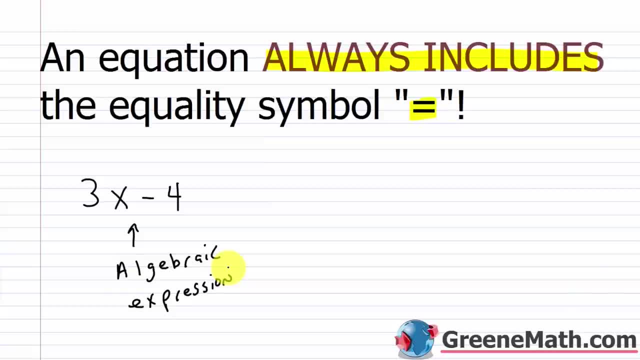 Sound: что там. let x equal 2. I could plug a 2 in there and I could evaluate, right, and in that particular case you might see an equal sign, because I'm saying, hey, if x equals 2, this algebraic expression is equal to this value, right, but it didn't start out with an equal sign, right? there's nothing there. 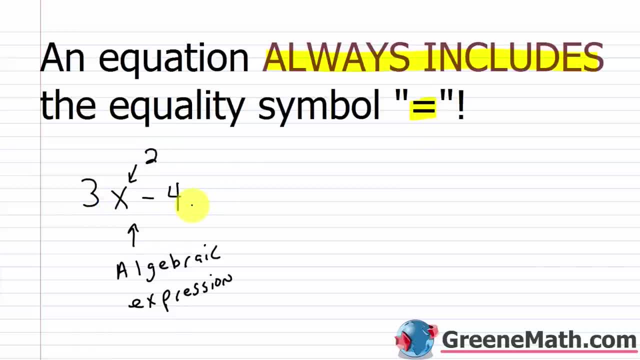 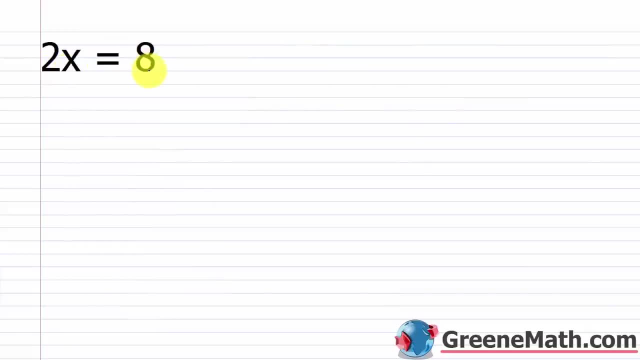 other than 3x minus 4 at this point. so that's an algebraic expression. an equation is going to look like this we have: 2x is equal to 8. so that's the main difference. if you're just starting out in algebra and you get a test and you see 2x equals 8, well okay, it has an equal sign to start. so this: 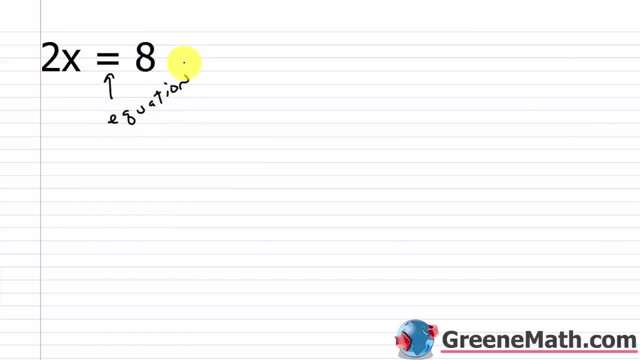 is an equation. this is an equation. that's your number one way to tell right, it's got an equal sign. it's an equation, you see, something like 7x squared minus 1. okay, no equal sign. this is an algebraic, algebraic expression. so let's talk a little bit about equations now, and we're not going to get to solving equations. 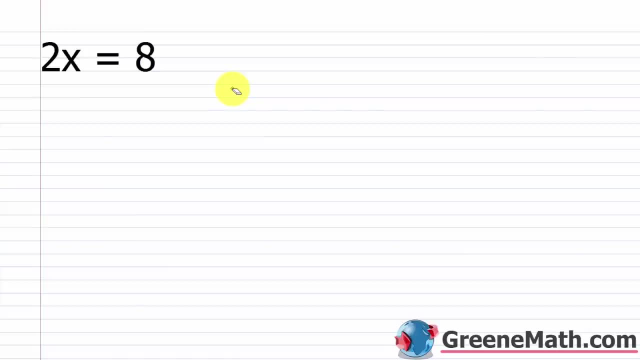 until the next lesson. we're just going to learn some of the basics of equations now, so that we can just kind of lightly introduce the concept to ourselves. all right, so we start out with this: 2x equals 8. so for an equation to be true, the left and the right side must be the same. 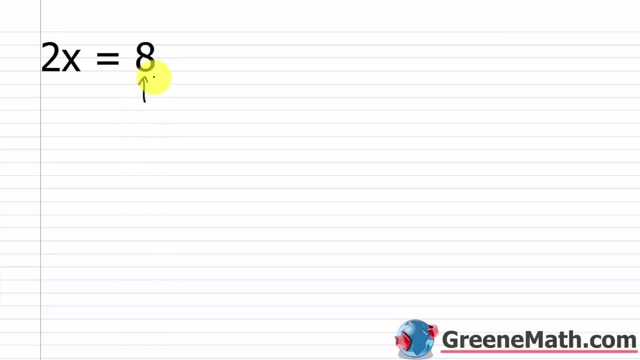 value. So if I look at the right side, the value is eight. it's just a number, the number eight. If I look at the left side, I have a two times x. I have two times x. So what you have to ask. 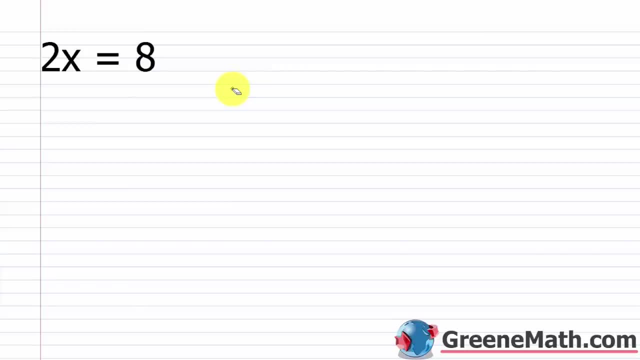 The concept to ourselves. All right, so we start out with this 2x equals 8. So for an equation to be true, the left and the right side must be the same value. So if I look at the right side, the value is 8. It's just a number, the number 8. If I look at the left side, I have a 2 times x. I have 2 times x. So what you have to ask yourself is what value, 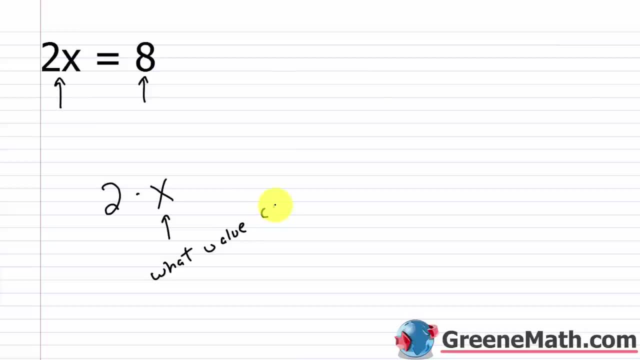 what value can I substitute to get a value of 8? 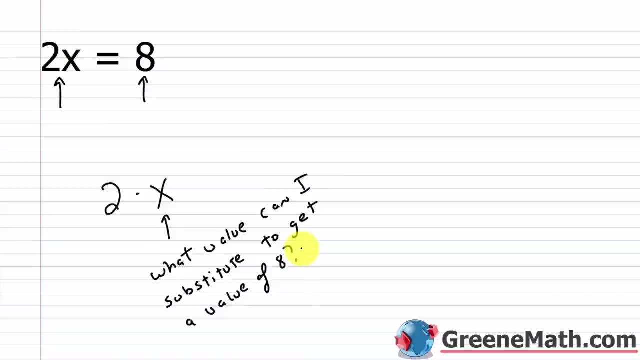 And why do I want a value of 8? Well, for an equation to be true, again, the left and the right side need to be equal. The right side is 8. The left side is 2 times x. So what I'm saying is 2 times some number is equal to 8. Now, can you think of a number that when you multiply by 2, 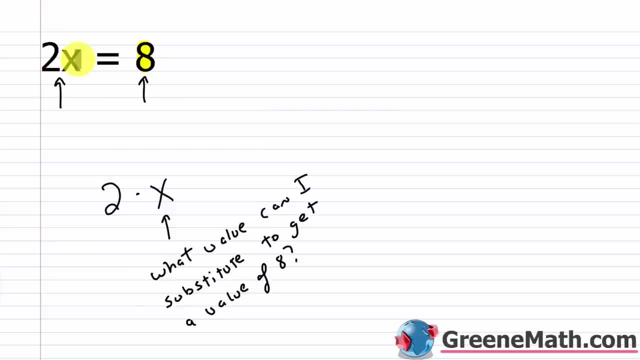 you get 8? And almost all of you know that that number is 4. So in other words, if I replace x with 4, I get a true statement, meaning the left and the right side would both be 8, right? They'd both be the same value. So this is true, true if x equals 4. 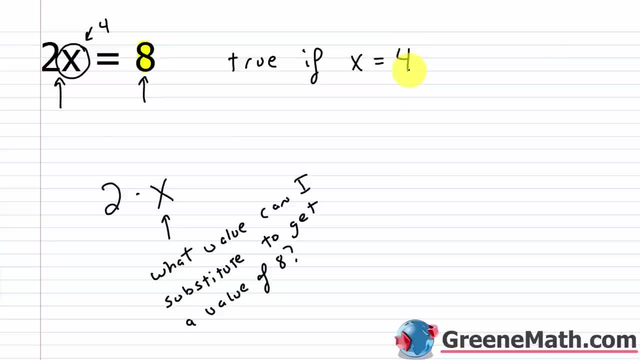 And the way you check it is you just plug in, just like we did in the last lesson when we're talking about algebraic expressions. Now we're kind of carrying that over. We're going to plug in a 4 for x, and we're going to see if the left and the right side are equal. So 2 times 4 should be equal to 8. And of course it is. 8 equals 8. And when you do this type of replacement, you're just looking for the same value on both sides. So 8 and 8, that checks out. If I had replaced x with anything else, I would have gotten a false statement. And the reason for that is there's no other number that when you multiply by 2, you get 8, right? It doesn't exist. So if I was to pick, let's say 3, for example. Let's say I said that x was equal to 3. Well, 2 times 3 is not equal to 8, right? I'd get 6 equals 8. That doesn't make any sense, right? 6 and 8 are not the same. They're not equal. So this is wrong. 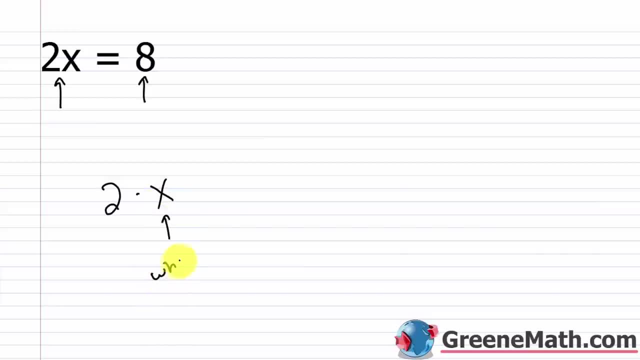 yourself is: what value? what value can I substitute to get a value of eight? And why do I want a value of eight? Well, for an equation to be true again, the left and the right side need to be equal. The right side is eight. 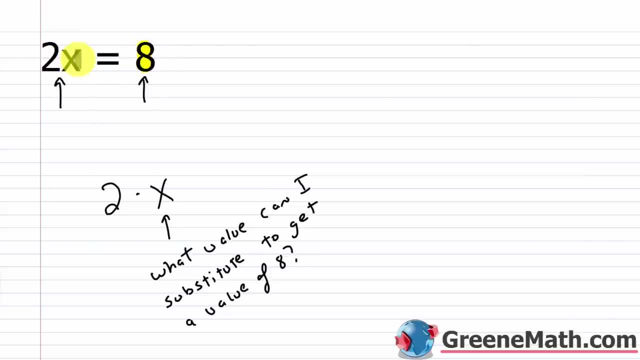 The left side is eight, The left side is eight. The left side is two times x. So what I'm saying is: two times some number is equal to eight. Now can you think of a number that when you multiply by two, you get eight? 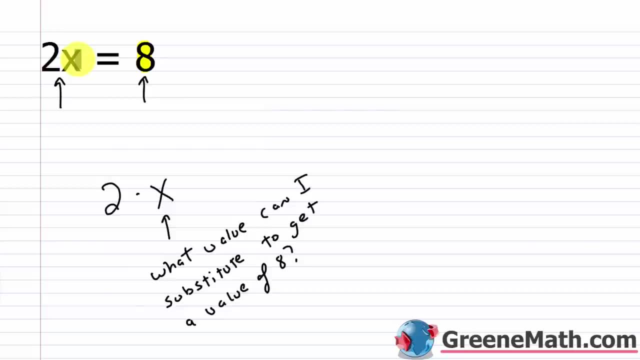 And almost all of you know that that number is four. So, in other words, if I replace x with four, I get a true statement meaning the left and the right side would both be eight right, They'd both be the same value. So this is true, true. 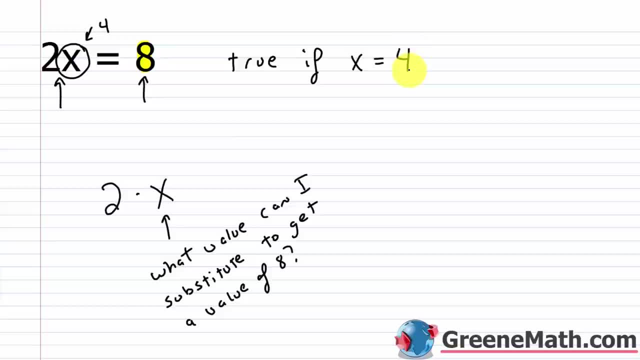 If x equals four. And the way you check it is you just plug in, just like we did in the last lesson when we're talking about algebraic expressions. Now we're kind of carrying that over. We're going to plug in a four for x And we're going to see if the left and the right side are equal, So two. 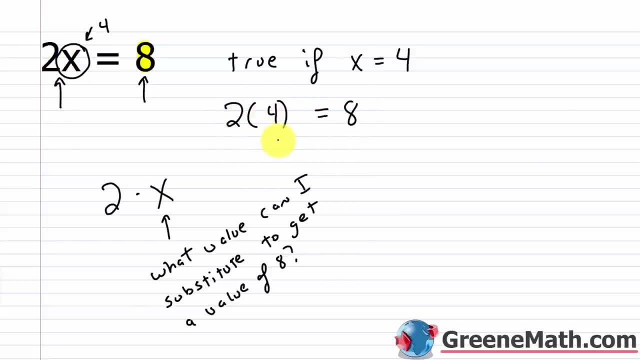 times four should be equal to eight, And of course it is eight equals eight, And when you do this type of replacement you're just looking for the same value on both sides. So eight and eight. that checks out. If I had replaced x with anything else, I would have gotten a false statement. 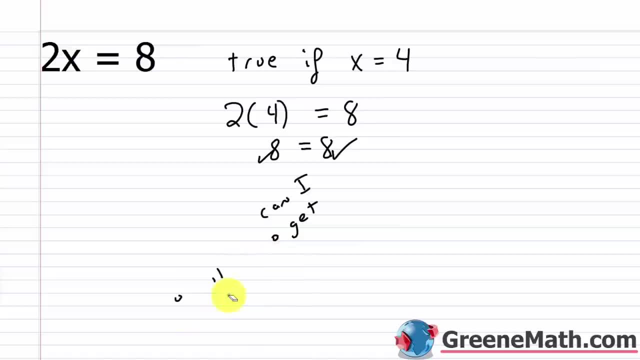 And the reason for that is there's no other number that when you multiply by two you get eight. right, It doesn't exist. So if I was to pick, let's say three, for example. let's say I said that x was equal to three. Well, two times three is not equal to eight. 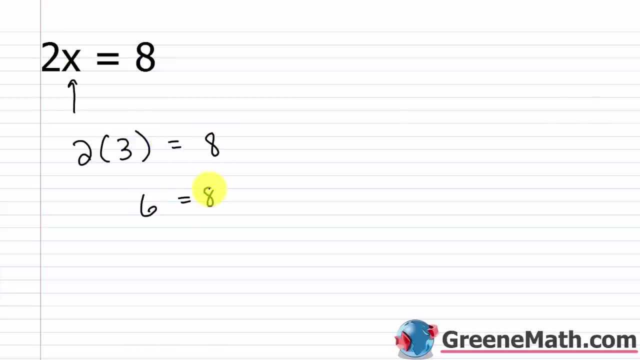 right, I'd get six equals eight. That doesn't make any sense, right? Six and eight are not the same, They're not equal. So this is wrong. That's wrong. Okay, so you're looking for the value for that variable. that. 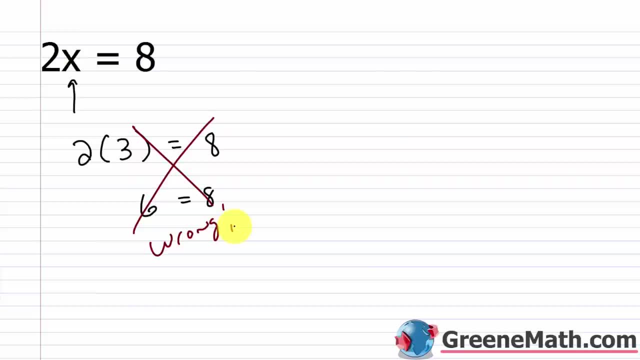 That's wrong. Okay. So you're looking for the value for that variable that makes the equation true, meaning the left and the right side will be the same. In this case, that's going to be 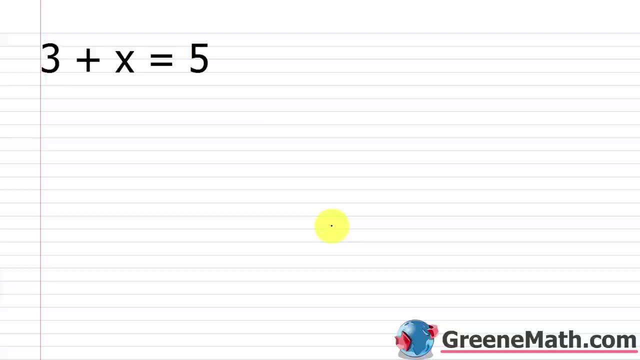 x equals 4. All right. So now let's look at 3 plus x equals 5. So again, I want a value for x 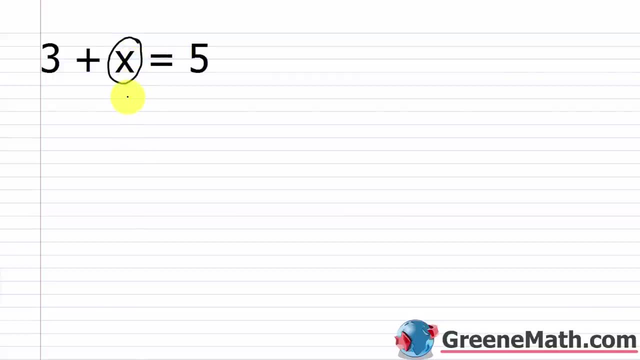 that when I substitute it for x, I get a true statement. So 3 plus what? 3 plus question mark gives me 5. Gives me 5. That's what I'm looking for. 3 plus what gives 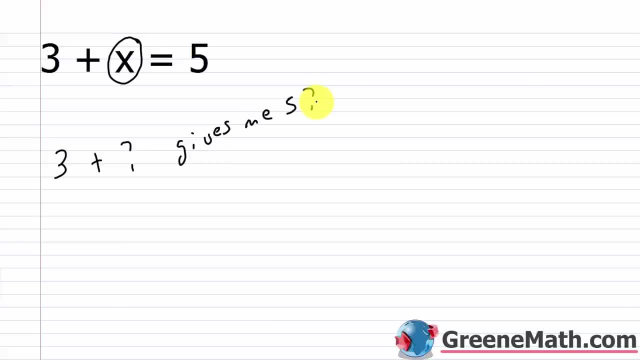 me 5? Well, we all know that that answer is 2. So if x is equal to 2, I get a true statement, 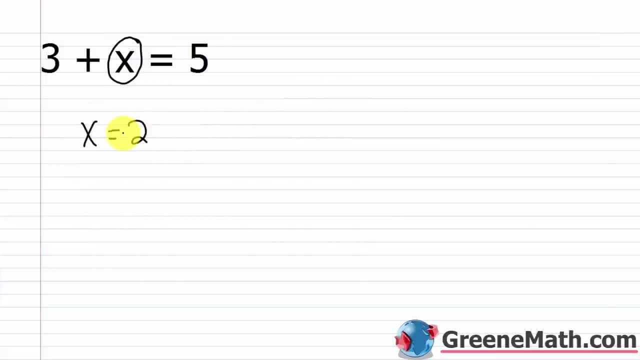 right? If x equals 2, this equation is true. And again, just plug in for the x. So 3 plus 2 is equal to 5. The left side will become 5. 3 plus 2 is 5. And that equals 5. I'm looking for the same thing. I'm looking for the same thing. I'm looking for the same thing. I'm looking for 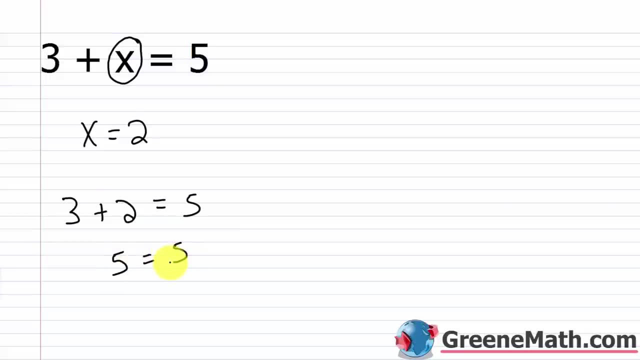 the same value on the left and the right side of the equation, okay? If I would choose any other 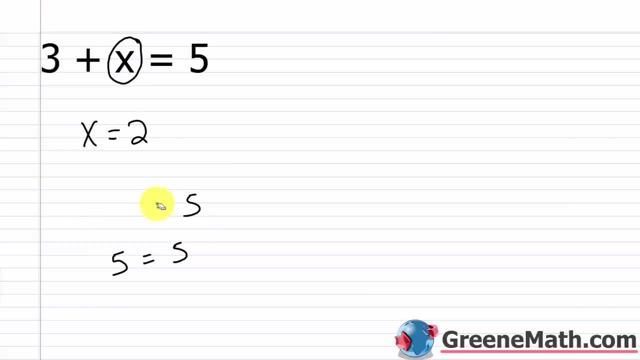 number here, I would get a false statement. Let's say, for example, I said that x was equal to, I don't know, negative 1. So if I plugged in a negative 1 for x, I put 3 plus negative 1 equals 5. 3 plus negative 1 is 2. So I'd have 2 equals 5. So if you solve an equation and the left and the right side are not equal, you didn't get a true statement. So if you solve an equation and the left and the right side are not equal, you did something wrong, right? You need the left 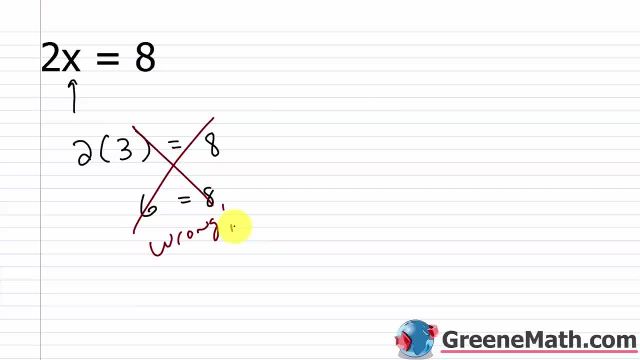 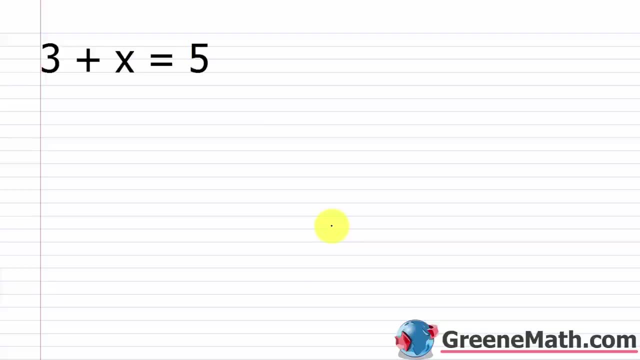 makes the equation true, meaning the left and the right side will be the same. In this case that's going to be x equals four, All right, so now let's look at: three plus x equals five. So again, I want a value for x, that when I substitute it for x, I get a true statement. So 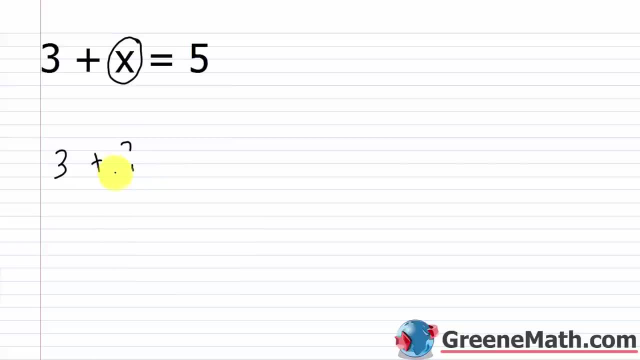 three plus what? three plus question mark gives me five, gives me five. That's what I'm looking for. Three plus what gives me five? Well, we all know that that answer is two. So if x is equal to two, I get a true statement, right? If x equals two, this equation is true. And again, just plug. 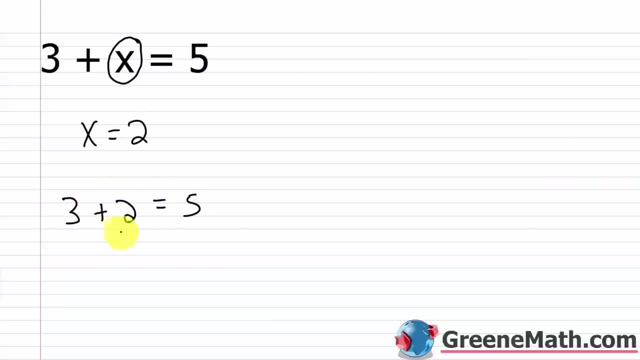 in for the x. So three plus two is equal to five. The left side will become five. three plus two is five, and that equals five. I'm looking for the same value on the left and the right side of the equation. okay, If I would choose any other number here, I would get a false. 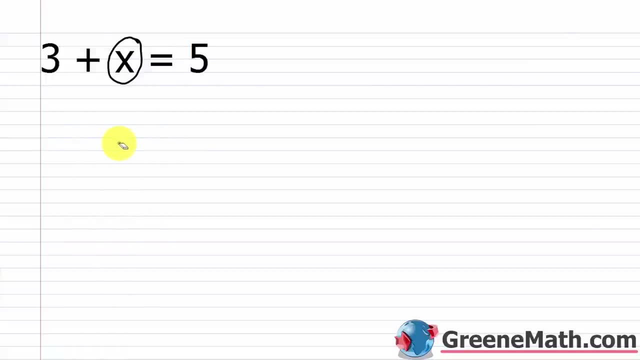 statement. Let's say, for example, I said that x was equal to- I don't know negative one. So if I plugged in a negative one for x, I put: three plus negative one equals five. Three plus negative one is two, So I'd have two equals five. So if you solve an equation, you're going to get a true. 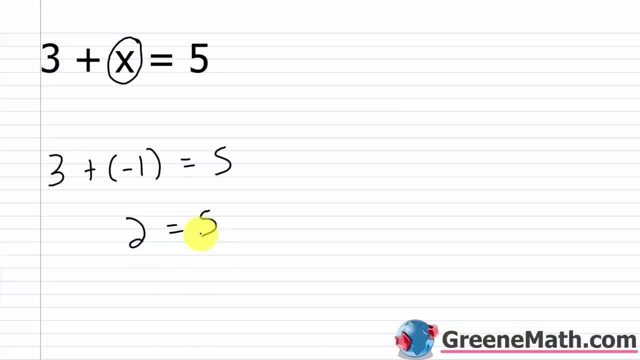 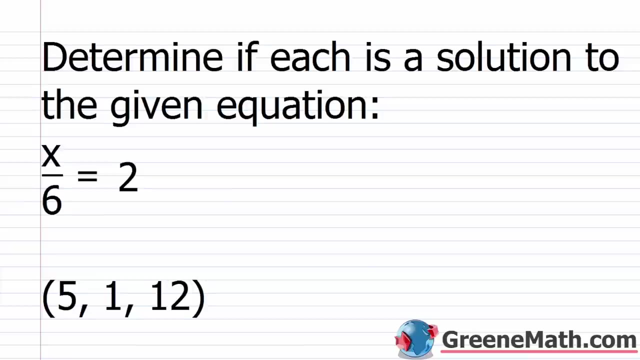 statement. So if you did something wrong, right, You need the left and the right side to be the same. This is wrong, wrong. The only value for x that's going to work is two right, Because three plus two is going to give us five. All right, let's take a look at a little practice exercise. 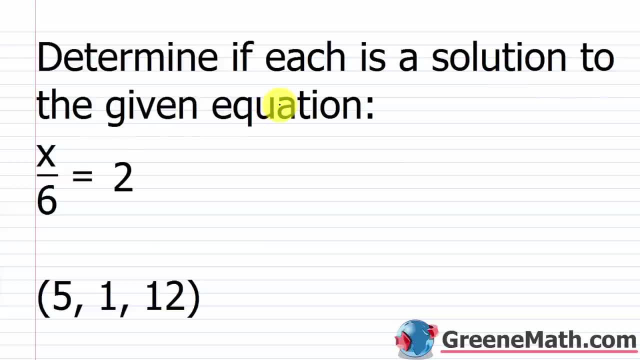 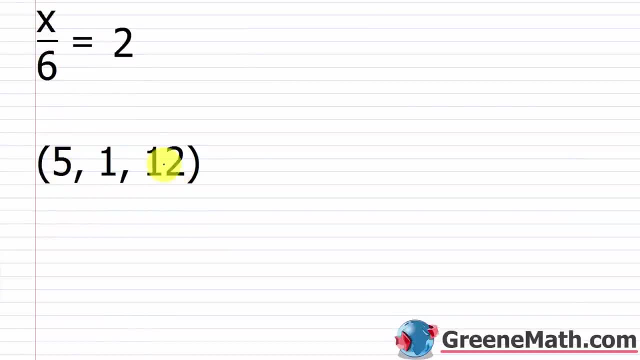 We want to determine if each is a solution to the given equation. So we're going to start out with x over six is equal to two, And then here are the values that we're going to use to solve the given equation, that we're going to try out as solutions. So let me kind of write this down here. We have x. 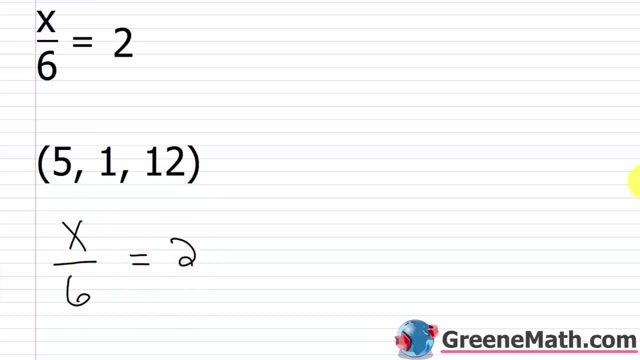 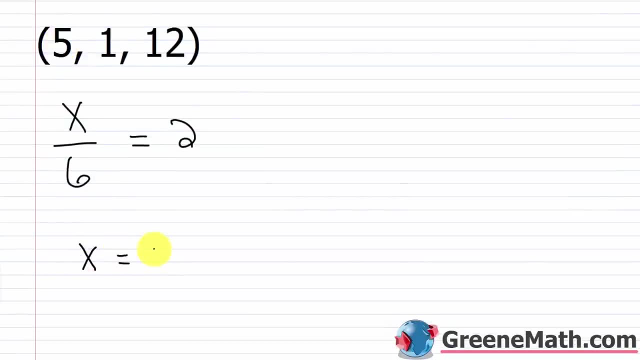 over six is equal to two. Let me scroll down and get a little room going. So I'm going to start out with the value of five. So I'm going to say: is x equals five? a solution? Well, to figure that out, I'm just going to plug a five in for x. So five plugged in for x over six, does that equal? 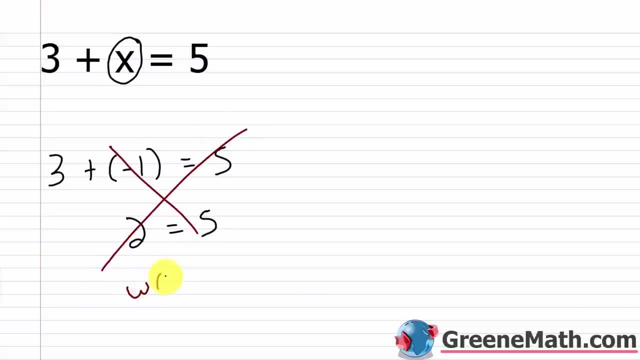 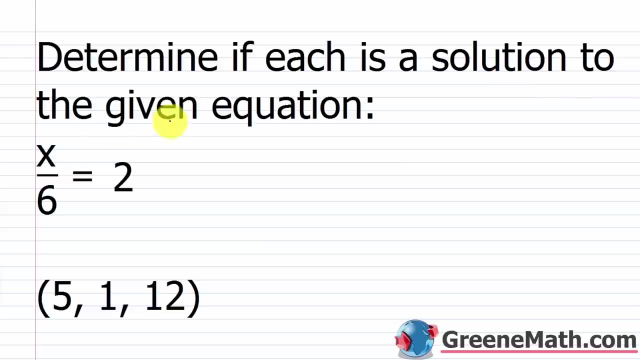 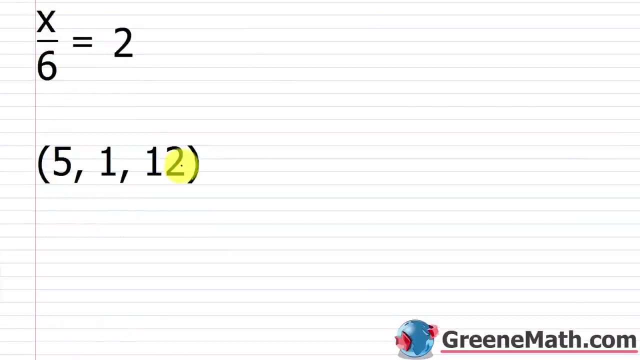 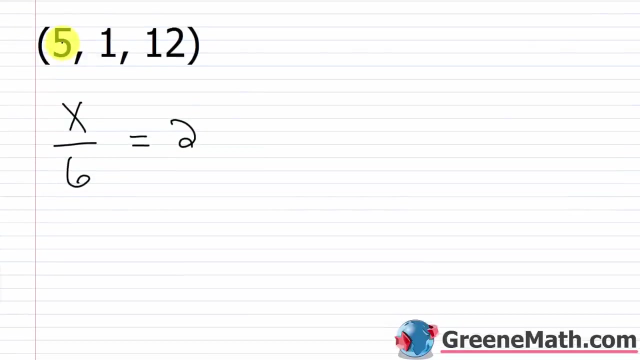 and the right side to be the same. This is wrong. Wrong. The only value for x that's going to work is 2, right? Because 3 plus 2 is going to give us 5. All right, let's take a look at a little practice exercise. We want to determine if each is a solution to the given equation. So we're going to start out with x over 6 is equal to 2. And then here are the values that we're going to try out as solutions. So let me kind of write this down here. We have x over 6 is equal to 2. Let me scroll down and get a little room going. So I'm going to start out with the value of 5. So I'm going to say, is x equals 5 a solution? Well, to figure that out, I'm just going to plug a 5 in for x. So 5 plugged in for x over 6, does that equal 2? No, it doesn't. All right, it doesn't. 5, 6 is less than 1, so it can't be equal to 2. 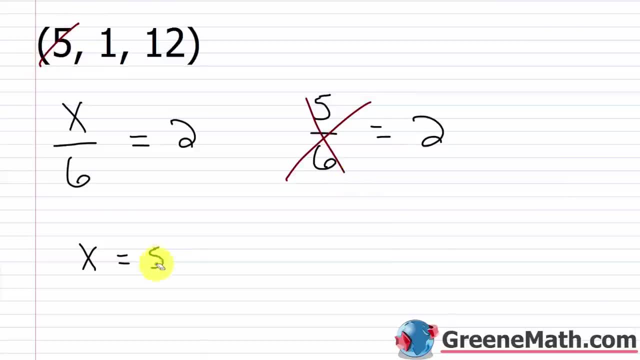 All right, so this doesn't work as a solution. Now, the next value they want us to try is 1. 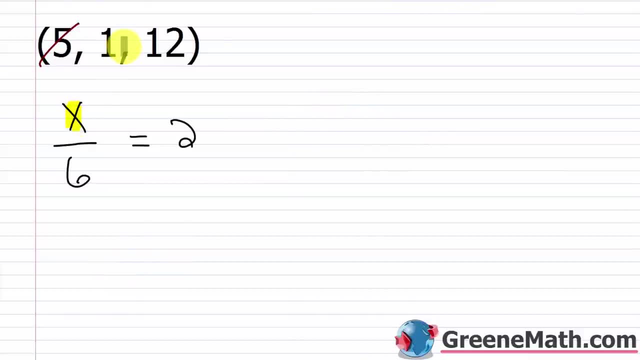 So I would plug a 1 in for x. I'm going to plug a 1 in there. 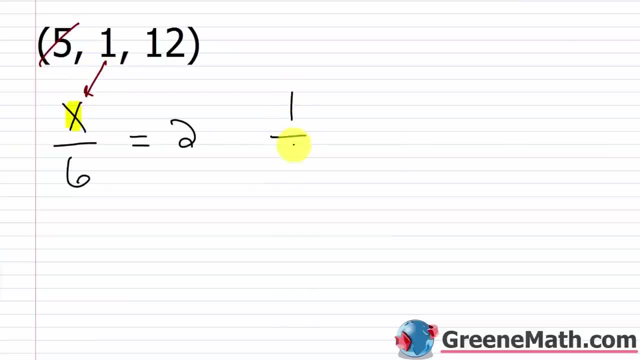 And I'm going to see if I get a true statement. So 1 over 6 is equal to 2. Is that true? Well, no, it's not. 1 sixth is not equal to 2. So that doesn't work as a solution either. 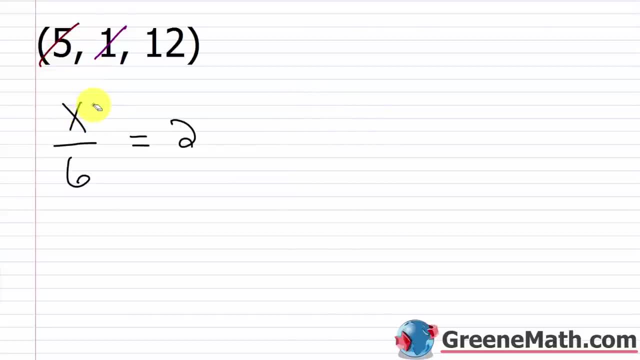 Let's try the last one. The last one is 12. 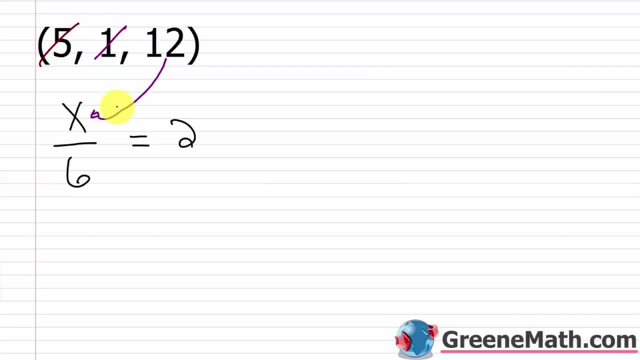 So I'm going to plug a 12 in for x now and see if that works out. So we would have 12 over 6 equals 2. Well, 12 over 6, that's 12 divided by 6. That is 2. So the left side is going to become 2. And the right side is 2. So the left and the right side are equal. They are the same value. And so, yes, 12 is a solution here. OK, 12 is a solution here. So we can say that x equals 12 is our answer. 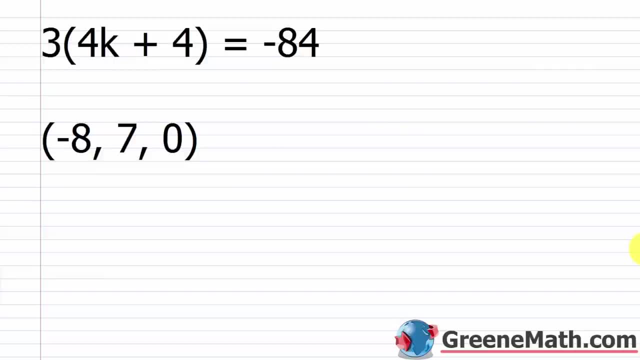 All right. So let's take a look at another one. We have 3 times the quantity 4k plus 4. And this is equal 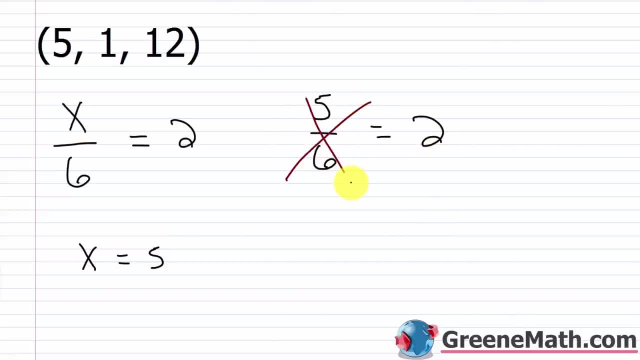 two: No, it doesn't. All right, it doesn't. Five. six is less than one, so it can't be equal to two, right? So this doesn't work as a solution. Now, the next value they want us to try is one. So I would plug a one in for x. I'm going to plug. 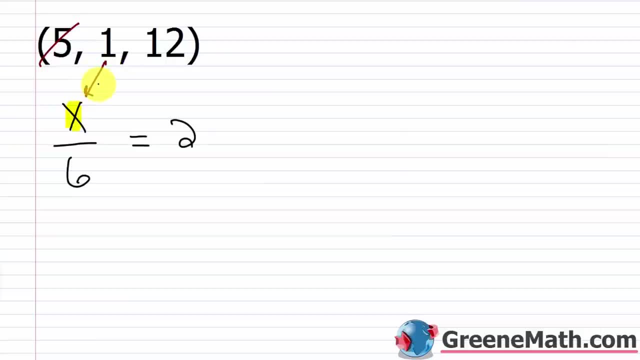 a one in there, And I'm going to see if I get a true statement. So one over six is equal to two, Is that true? Well, no, it's not. One sixth is not equal to two, So that doesn't work as a solution. 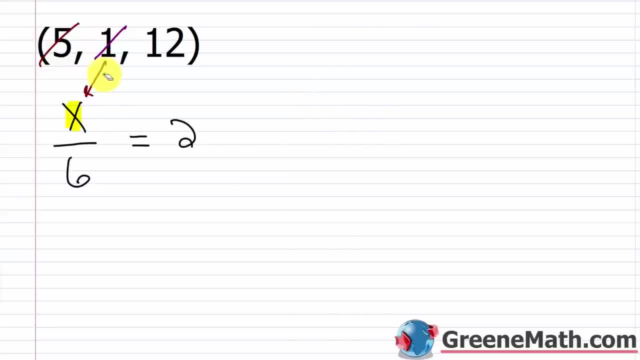 either. The last one is 12.. So I'm going to plug a 12 in for x now and see if that works out. So we would have: 12 over six equals two. Well, 12 over six, that's 12 divided by six, that is two. So the 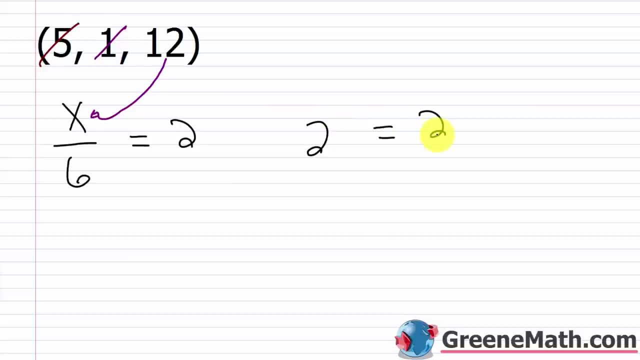 left side is going to become two and the right side is two, So the left and the right side are equal. they are the same value, And so, yes, 12 is a solution here. Okay, 12 is a solution here. 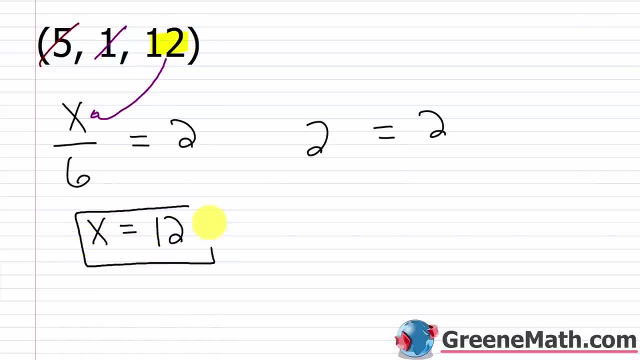 So we can say that x equals two. So we're going to plug a 12 in for x now and see if that works out. x equals 12 is our answer. All right, let's take a look at another one. We have three times the. 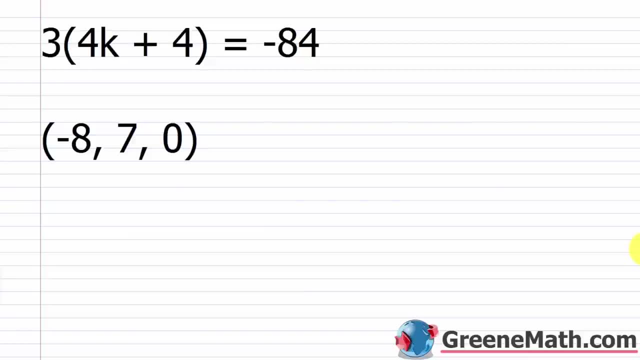 quantity 4k plus four, and this is equal to negative 84.. So again, what I'm going to do is take each value here and plug it in for our variable- in this case it's k- and see if we get a true statement, see if the left and the right side are equal. If we do, then we know that. 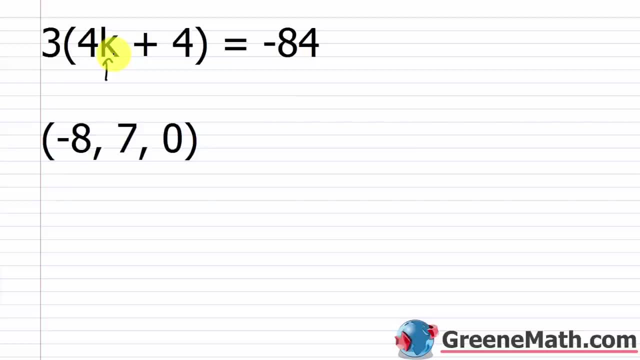 that value is a solution for the equation, right? So I'm going to start out with negative eight and I'm just going to plug it in for k, And so we'll have three times this quantity, four times negative eight, then plus four. 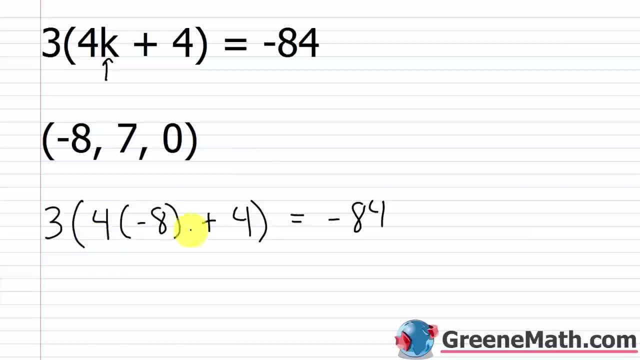 and this equals negative 84.. So I'm going to start out inside the parentheses with four times negative eight. that's negative 32.. Then when I'm done with that, I would continue inside the parentheses. I would add four negative 32 plus four is negative 28.. So this would be three. 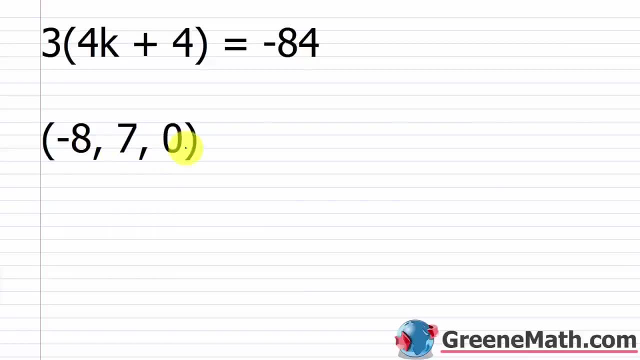 to negative 84. So again, what I'm going to do is take each value here and plug it in for our variable. In this case, it's k. And see if we get a true statement. See if the left and the right side are equal. If we do, then we know that that value is a solution for the equation. All right. 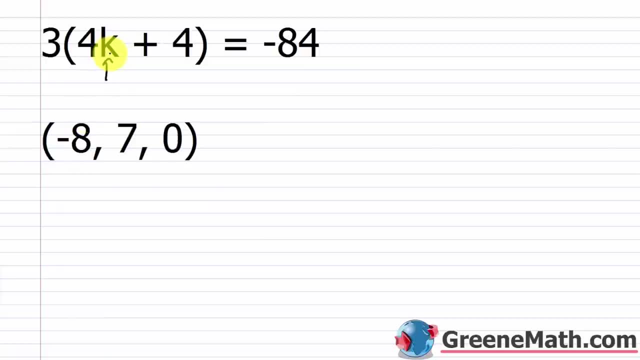 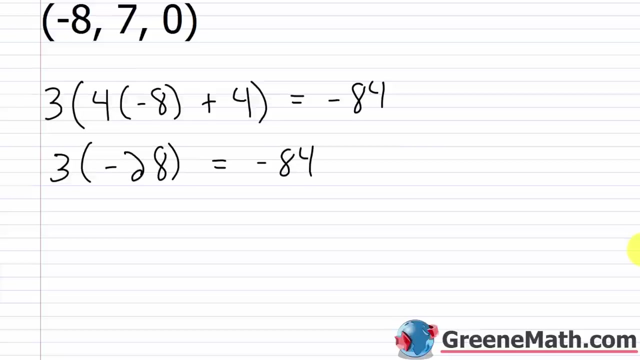 So I'm going to start out with negative 8. And I'm just going to plug it in for k. And so we'll get the quantity 4 times negative 8, then plus 4. And this equals negative 84. So I'm going to start out inside the parentheses with 4 times negative 8. That's negative 32. And then when I'm done with that, I would continue inside the parentheses. I would add 4. Negative 32 plus 4 is negative 28. So this would be 3 times negative 28. And this equals negative 84. All right. So I know that 3 times negative 28 would be negative. 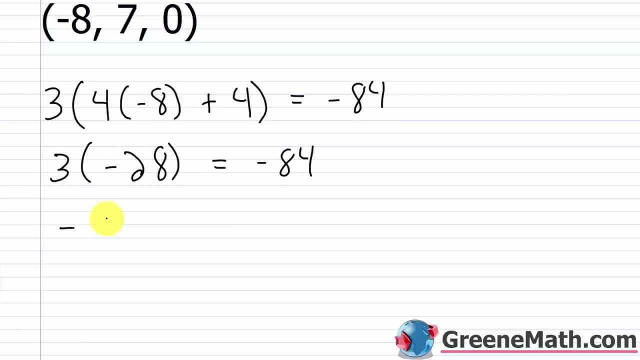 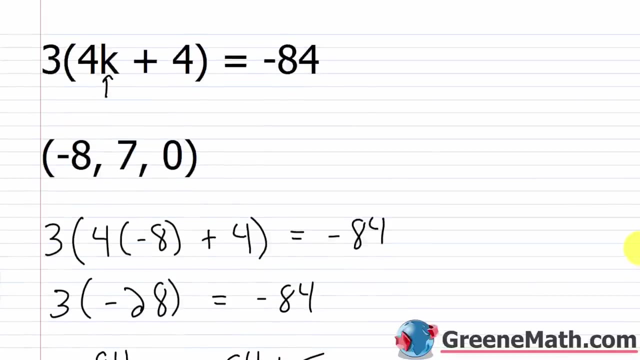 And then 3 times 20 is 60. 3 times 8 is 24. So 60 plus 24 is 84. So this would be negative 84 over here. And over here, it's negative 84. So that checks out. So negative 8 is a solution for this equation. Okay. This is a solution. Let's say k is equal to negative 8. Now, we'll try the other ones, but they're going to fail. So let's go ahead and erase this real quick. 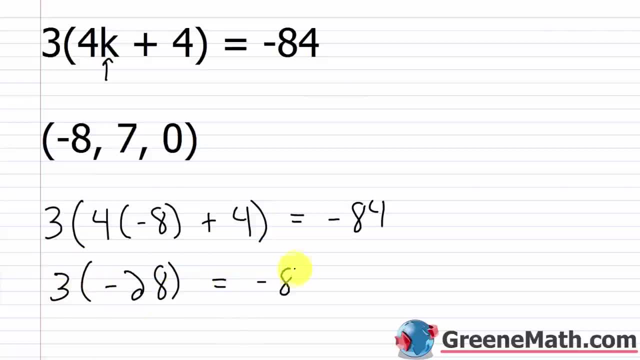 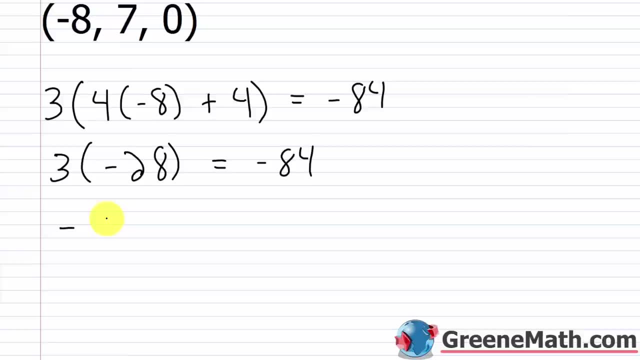 times negative 28. And this equals negative 84.. All right, I'm going to take my two values: three times negative 28 would be negative, and then three times 20 is 60.. Three times eight is 24.. So 60 plus 24 is 84. So this would be negative 84 over. 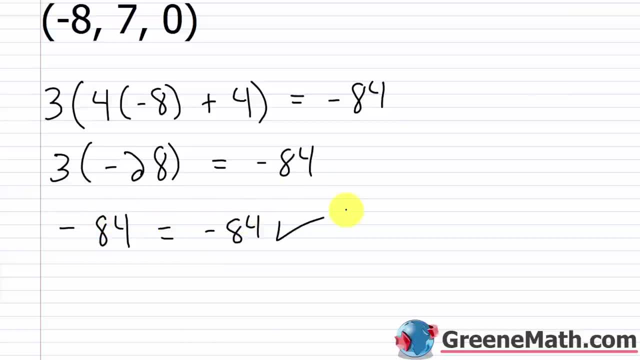 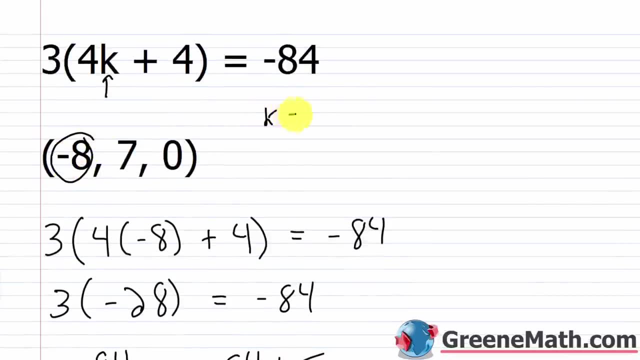 here And over here it's negative 84.. So that checks out. So negative eight is a solution for this equation. Okay, this is a solution. and say k is equal to negative eight. Now we'll try the other ones, but they're going to fail. 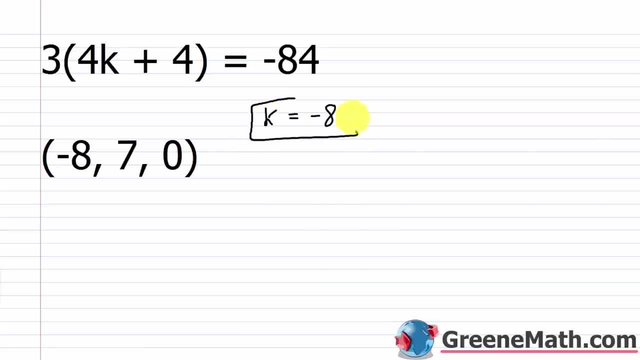 So let's go ahead and erase this real quick, Put a check mark right here. Let's go with seven. Let's see if that works out for us. So we're gonna put three times the quantity, four times, instead of K. I'm plugging in seven. 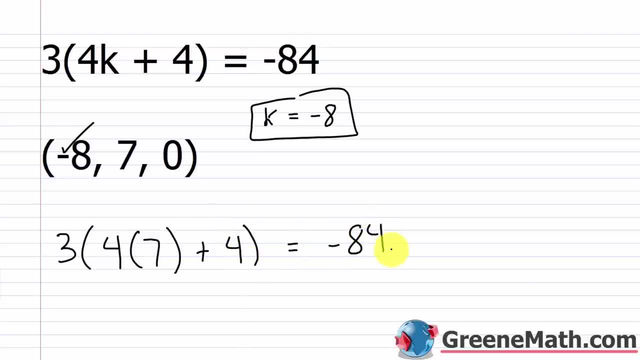 plus four equals negative 84.. Four times seven is 28,, then 28 plus four is 32.. So I'd have three times 32 and that's gonna equal negative 84.. Now, without doing the multiplication, I already know this isn't gonna work. 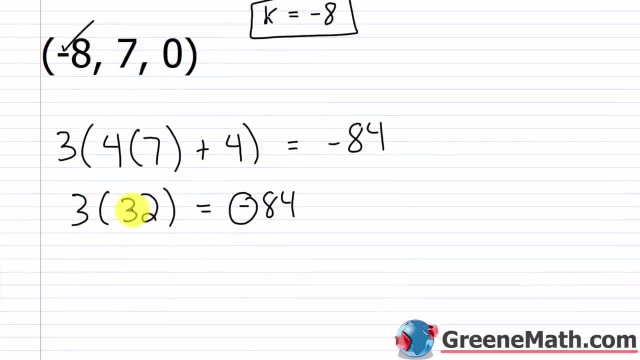 because this is negative over here and this is two positives being multiplied together. So even if the number part worked out- which it's not going to- we'd end up with a positive on one side and a negative on the other, so we know it's going to fail. 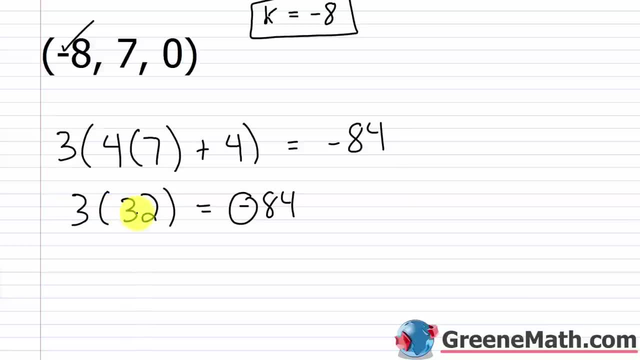 We can go ahead and say: well, what is three times 32?? Three times 30 is 90,, three times two is six, So this is 96, and that's not equal to negative 84. That's, that doesn't work, right. 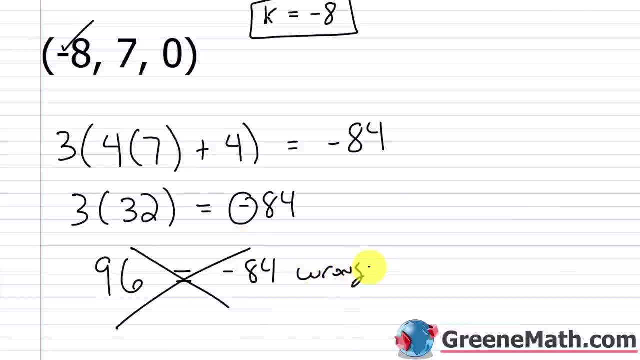 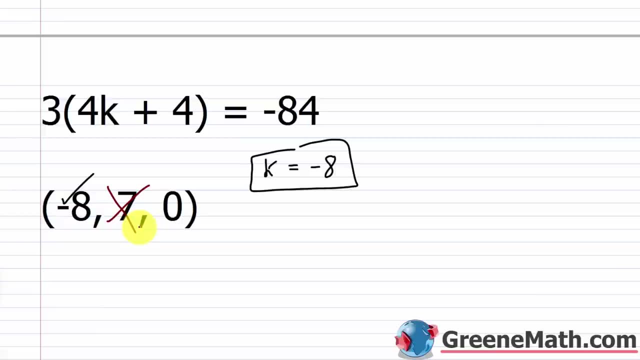 This is wrong. So seven is not a solution for the equation. You can go back up here and I'm gonna mark that out. That didn't work. Now, the last value we're gonna try is zero, So we're gonna plug in a zero for K. 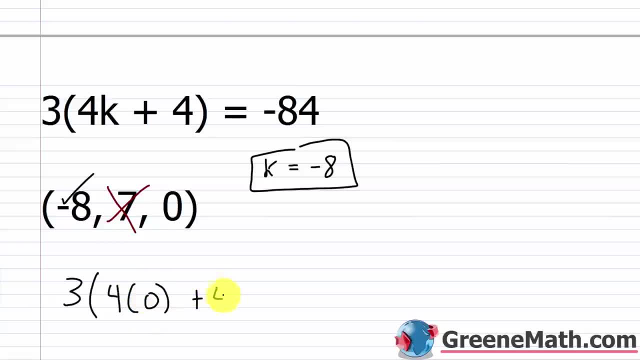 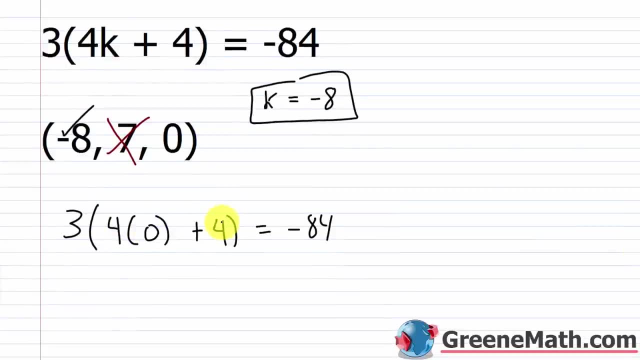 Three times this quantity, four times zero plus four, equals negative 84.. All right, so four times zero is zero, then zero plus four is four. So I'd have: three times four equals negative 84.. Three times four is equal to negative 84.. 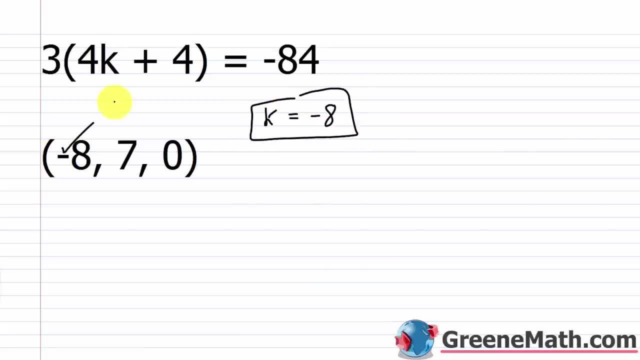 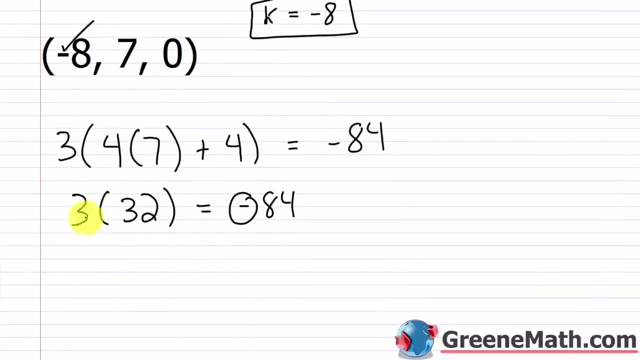 Put a check mark right here. Let's go with 7. Let's see if that works out for us. So we're going to put 3 times the quantity, 4 times, instead of k, I'm plugging in 7, plus 4 equals negative 84. 4 times 7 is 28. Then 28 plus 4 is 32. So I'd have 3 times 32. And that's going to equal negative 84. Now, without doing the multiplication, I already know this isn't going to work because this is going to be negative 84. So I'm going to put 3 times the quantity, this is negative over here. And this is two positives being multiplied together. So even if the number part worked out, which it's not going to, we'd end up with a positive on one side and a negative on the other. So we know it's going to fail. But we can go ahead and say, well, what is 3 times 32? 3 times 30 is 90. 3 times 2 is 6. So this is 96. And that's not equal to negative 84. That doesn't work, right? This is wrong. 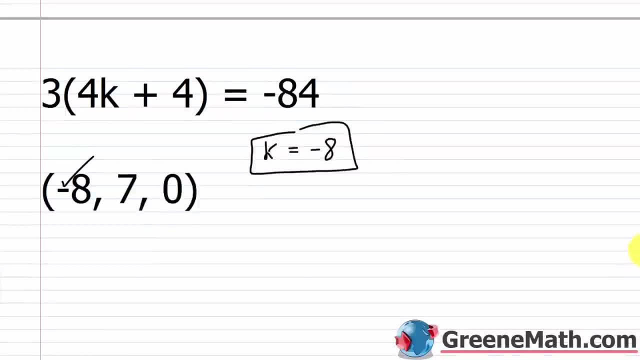 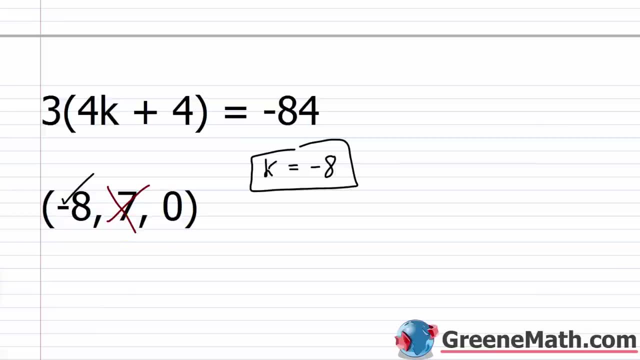 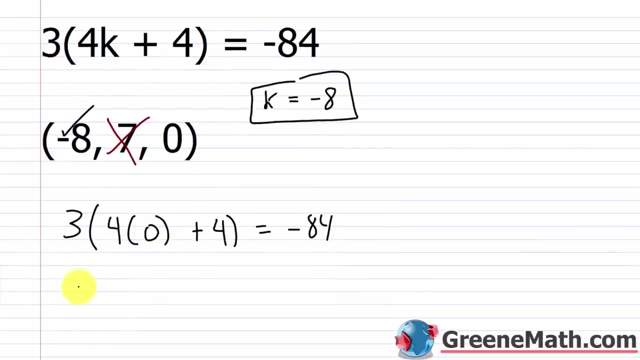 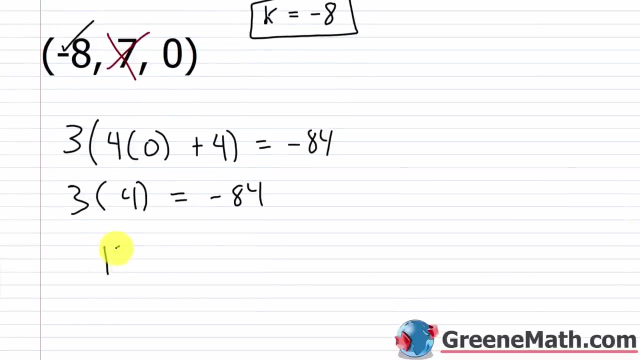 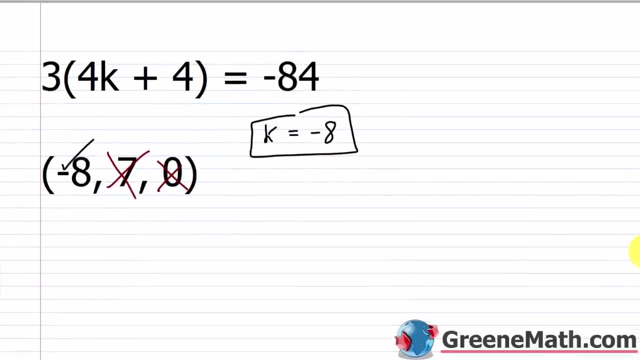 So 7 is not a solution for the equation. We can go back up here. And I'm going to mark that out. That didn't work. Now, the last value we're going to try is 0. So we're going to plug in a 0 for k. 3 times this quantity, 4 times 0, plus 4 equals negative 84. All right. So 4 times 0 is 0. Then 0 plus 4 is 4. So I'd have 3 times 4 is equal to negative 84. And obviously, it's not going to work. 3 times 4 is 12. And that does not equal negative 84. So the left and the right side are not the same value. I have negative 84 on the right. I have 12 on the left. Not the same. So this doesn't work. This is wrong. And so 0 is not a solution. So we saw that only k equals negative 8 is what works in our equation, right? And it works because when we plug in a negative 8 we get the same value on the left and on the right side. Again, that value was negative 84. 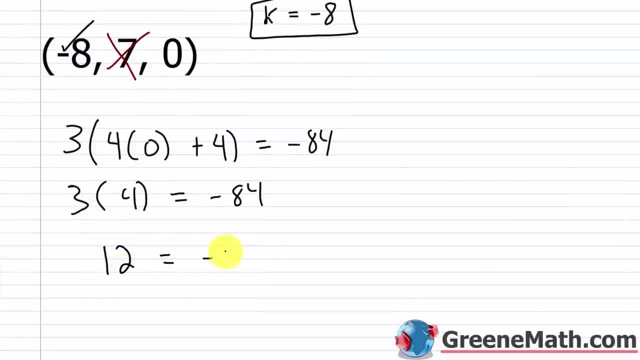 And obviously that's not gonna work. Three times four is 12, and that does not equal negative 84. So the left and the right side are not the same value. right, I have negative 84. on the right, I have 12 on the left, not the same. 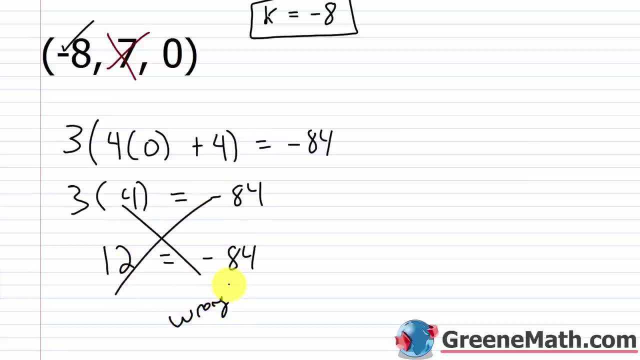 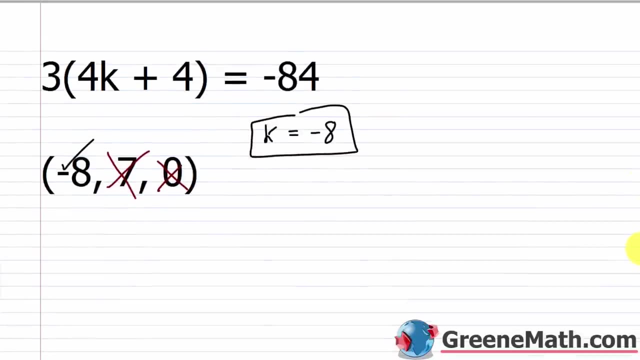 So this doesn't work, This is wrong, And so zero is not a solution. So we saw that only K equals negative eight is what works in our equation Right, and it works because when we plug in a negative eight for K, we get the same value on the left. 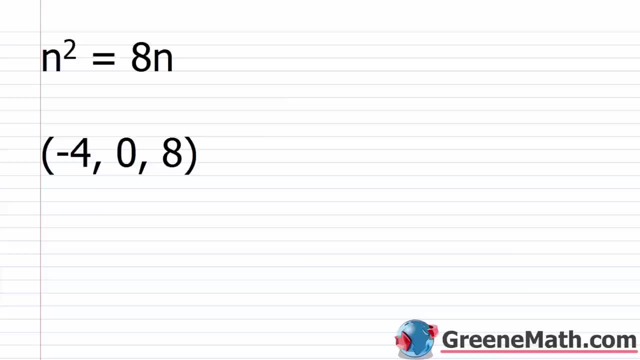 and on the right side. Again, that value was negative 84.. All right, let's take a look at another one. We have N, squared equals eight N. So here's our proposed solutions: We have negative four, we have zero and we have eight. 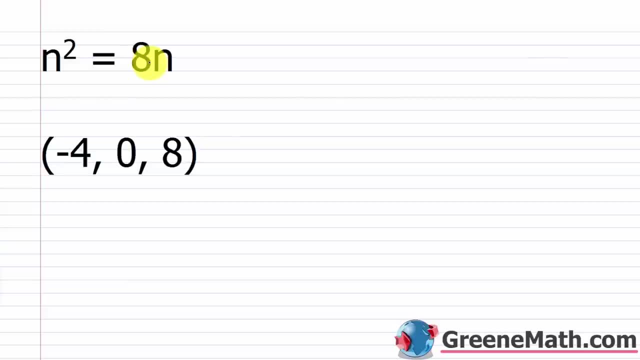 So let's start out with negative four, So I'm gonna plug that in. everywhere I see an N, You have to be careful, because in a lot of cases we're just plugging in one, And once here we have two Ns that we need to plug in for. 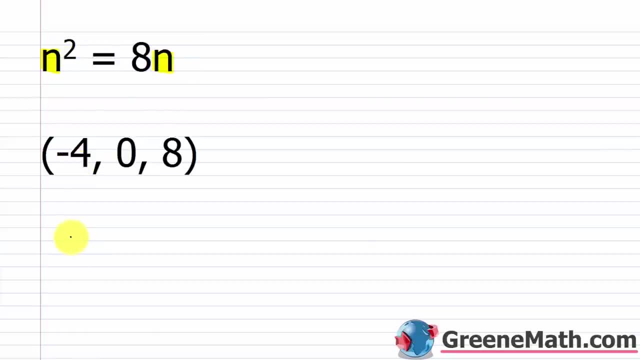 We have to plug in there and also there. I'm gonna start out by putting parentheses around negative four and then I'm gonna square that And this equals eight times negative four. Notice how I use parentheses when I'm substituting N- Very important here, because I have a negative number. 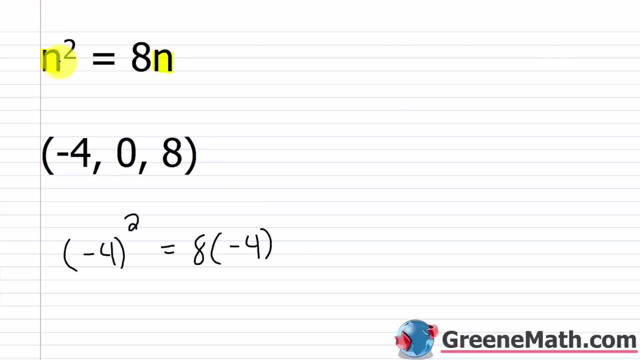 that is raised to a power, And I don't wanna make a sign mistake right. Whatever value I have for N in this case, that's negative four. I wanna square it, So I need to make sure I use parentheses. Okay, so negative four squared is gonna be positive 16.. 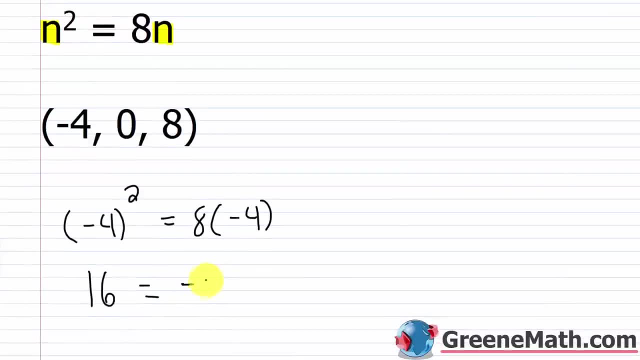 We're saying this is equal to eight times negative four, which is negative 32.. This obviously does not work out, And so this is not a solution, right? Negative four doesn't work. Let's try zero, So I would plug in a zero for N. 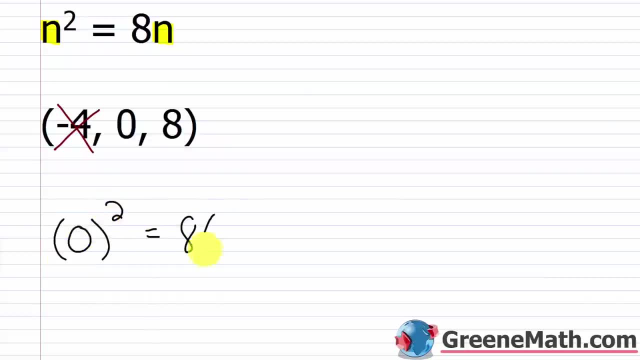 So I'd have: zero squared equals eight times zero. What's that gonna work as a solution? Zero squared is zero and eight times zero is also zero, So the same value occurs on the left and the right side. That value is zero, and so this is a solution, right. 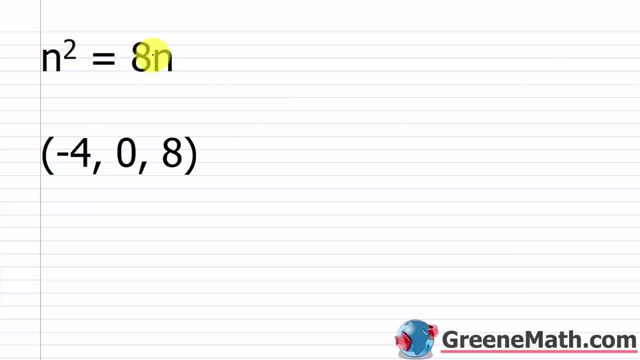 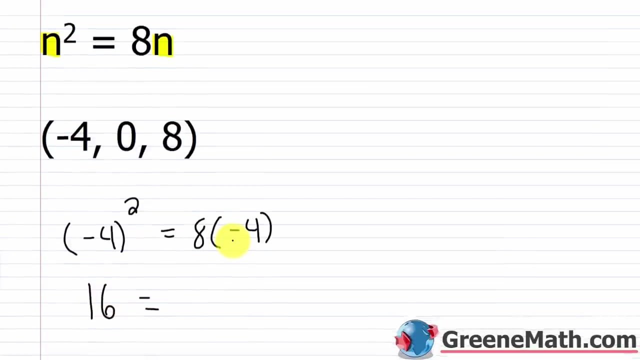 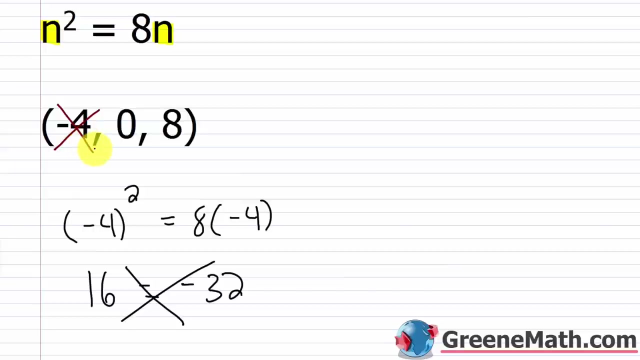 All right. Let's take a look at another one. We have n squared equals 8n. So here's our proposed solutions. We have negative 4. We have 0. And we have 8. So let's start out with negative 4. So I'm going to plug that in everywhere I see an n. You have to be careful because in a lot of cases, we're just plugging in once. Here we have two n's that we need to plug in for. We have to plug in so there. I'm going to start out by putting parentheses around negative 4. And then I'm going to square that. And this equals 8 times negative 4. Notice how I use parentheses when I'm substituting n. Very important here because I have a negative number that is raised to a power. And I don't want to make a sign mistake, right? Whatever value I have for n, in this case that's negative 4, I want to square it. So I need to make sure I use parentheses. Okay. So negative 4, square. I'm going to put a negative number that is raised to a power. And I don't want to make a sign mistake. So I'm going to put a negative number that is raised to a power. And I don't want to make is going to be positive 16. And we're saying this is equal to 8 times negative 4, which is negative 32. This obviously does not work out. And so this is not a solution, right? Negative 4 doesn't work. Let's try 0. So I would plug in a 0 for n. So I'd have 0 squared equals 8 times 0. And that is in fact going to work as a solution. 0 squared is 0. 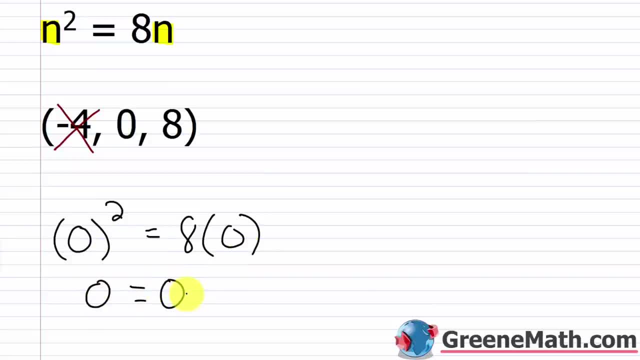 And 8 times 0 is also 0. So the same thing is going to work as a solution. So I'm going to same value occurs on the left and the right side that value is zero and so this is a solution right this is a solution all right let's try eight now so we have eight that we're plugging in for n that's going to be squared and then this is equal to eight times eight so eight squared is eight times eight that's 64 and this is equal to eight times eight that's 64 so that works also we get 64 equals 64 so eight is also a solution to 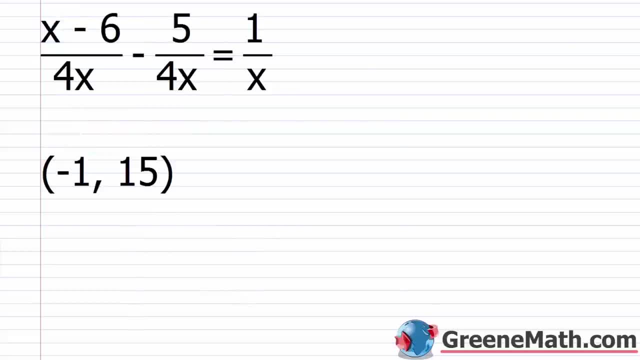 the equation all right let's take a look at one last problem so we have x minus six over four x minus five over four x equals one over x so we have a lot of places we need to plug into so I have two proposed solutions I have negative one and then I have 15 so for negative one I have one and I have 15. so for negative one I have negative one and then I have 15. 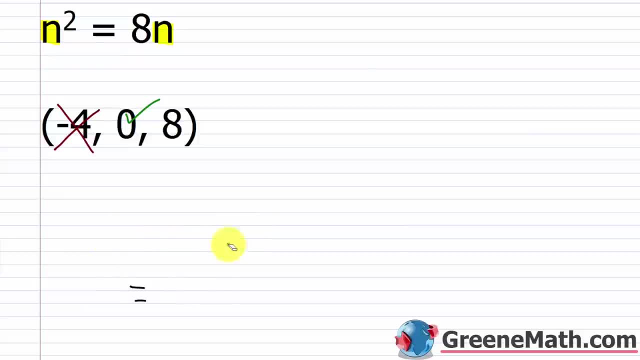 This is a solution. All right, let's try eight now. So we have eight that we're plugging in for N. that's gonna be squared, and then this is equal to eight times eight. So eight squared is eight times eight. That's gonna be eight squared. 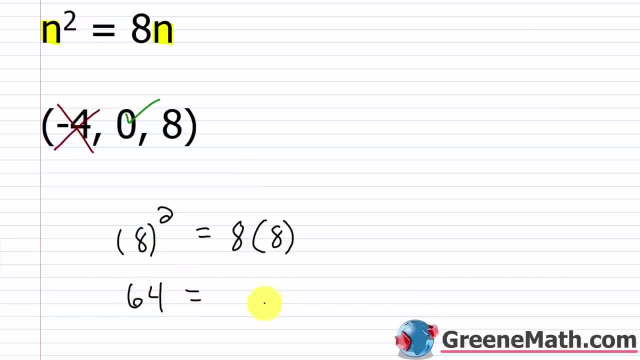 That's gonna be eight times eight, That's 64. And this is equal to eight times eight, That's 64. So that works also. We get 64 equals 64. So eight is also a solution to the equation. All right, let's take a look at one last problem. 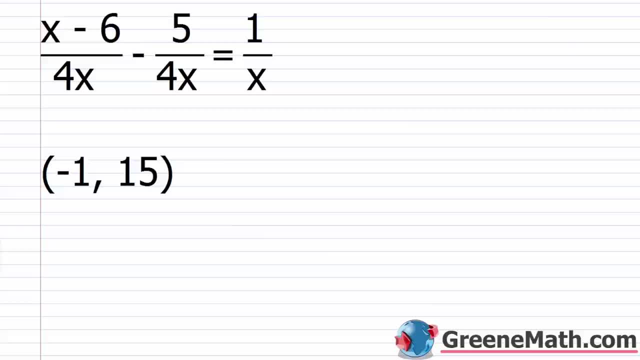 So we have X minus six over four, X minus five over four. X equals one over X. So we have a lot of places we need to plug into. So I have two proposed solutions. I have negative one and then I have 15.. So for negative one: 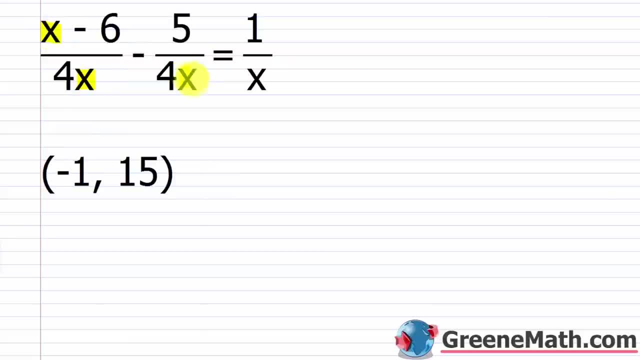 we're gonna plug that in here, here, here and here, So everywhere there's an X. So I would have negative one minus six over four times negative one, then minus five over four times negative one, And this should be equal to one over negative one. 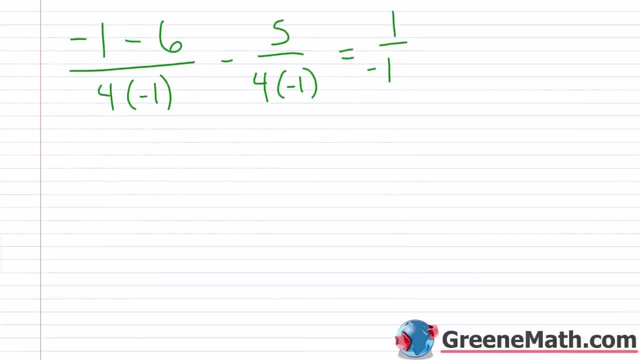 So let's crank this out real quick. So negative one minus six is negative seven, So that's negative seven over four times negative one, That's negative four. Then we're subtracting away, We have five over four times negative. one is negative four. 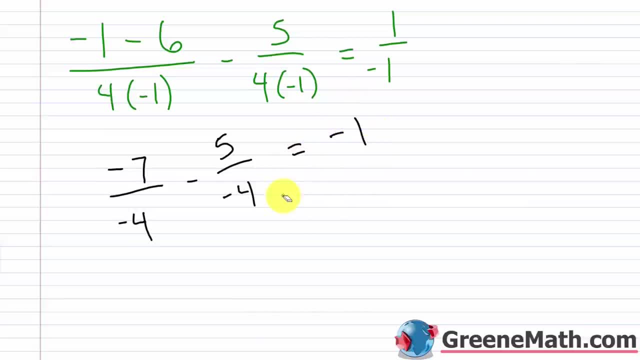 And this should be equal to one over negative one which is negative one. So if we look, we have a common denominator right now, And so we can just say what is negative: seven minus five. I just work with the numerators. 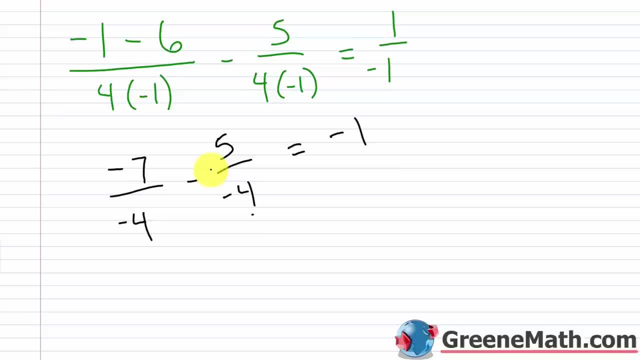 Well, negative seven minus five is negative 12.. And so if I had negative 12 over negative four, negative 12 over negative four, that's positive three, That's positive three. Positive three is not equal to negative one, So this does not work. 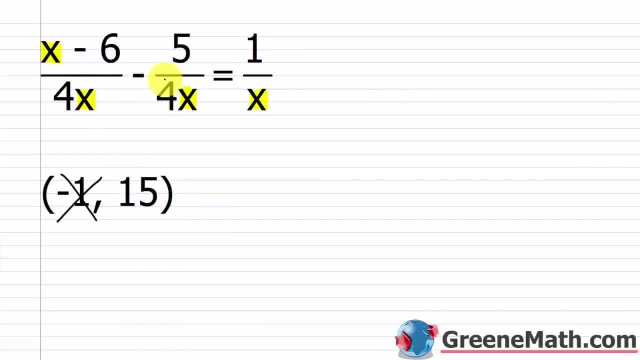 All right, let's try 15 now And again. everywhere I see an X, I'm gonna plug in a 15.. So I'd have 15 minus six over four times 15.. Then minus five over four times 15.. 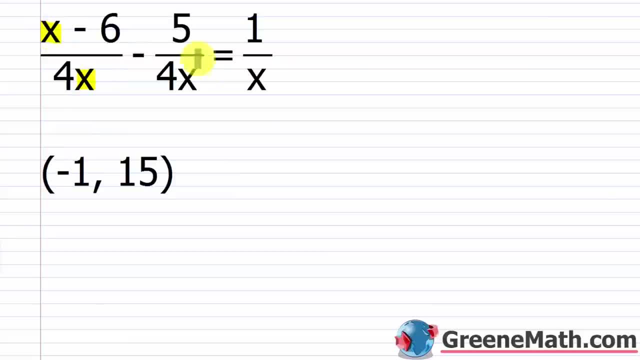 We're going to plug that in here, here, here, and here. So everywhere there's an x. 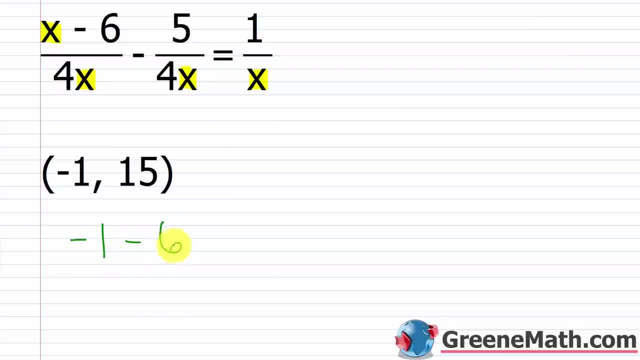 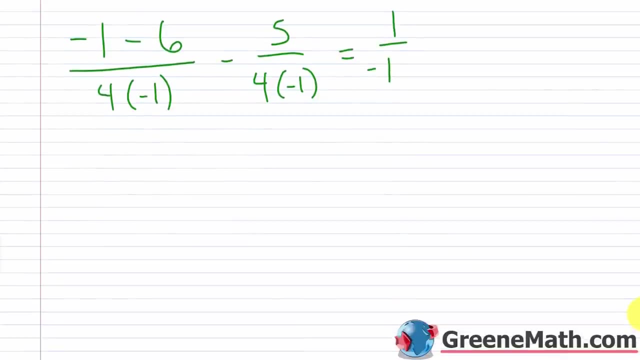 So I would have negative 1 minus 6 over 4 times negative 1. Then minus 5 over 4 times negative 1. And this should be equal to 1 over negative 1. So let's crank this out real quick. So negative 1 minus 6 is negative 7. So that's negative 7 over 4 times negative 1. That's negative 4. Then we're subtracting away. 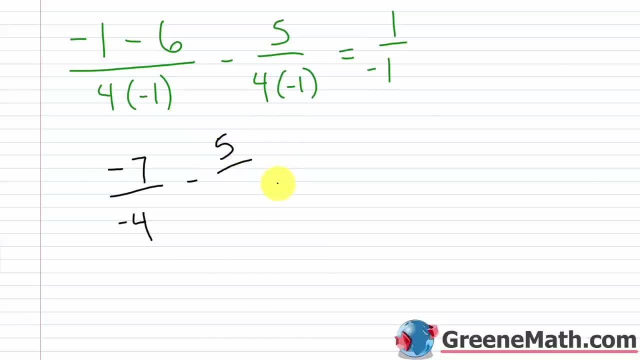 We have 5 over 4 times negative 1 is negative 4. And this should be equal to 1 over negative 1, which is negative 1. So if we look, we have a common denominator right now. And so we can just say, what is negative 7 minus 5? I just work with the numerators. Well, negative 7 minus 5 is negative 12. And so if I had negative 7 minus 5, negative 12 over negative 4, negative 12 over negative 4, that's positive 3. 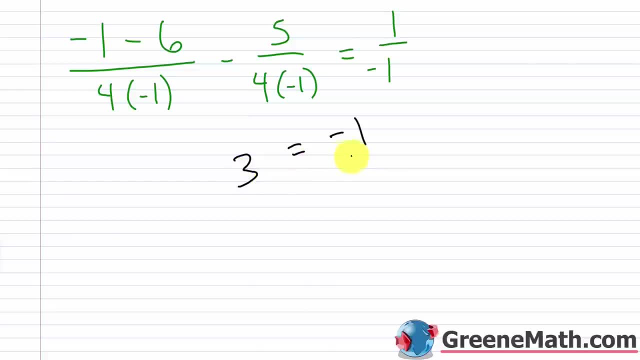 That's positive 3. Positive 3 is not equal to negative 1. So this does not work. 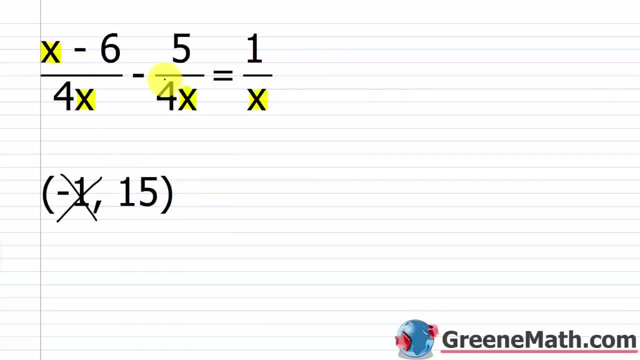 All right, let's try 15 now. And again, everywhere I see an x, I'm going to plug in a 15. So I'd have 15 minus 6 over 4 times 15. Then minus 5 over 4 times 15. This should be equal to 1 over 15. So let's crank this out real quick. 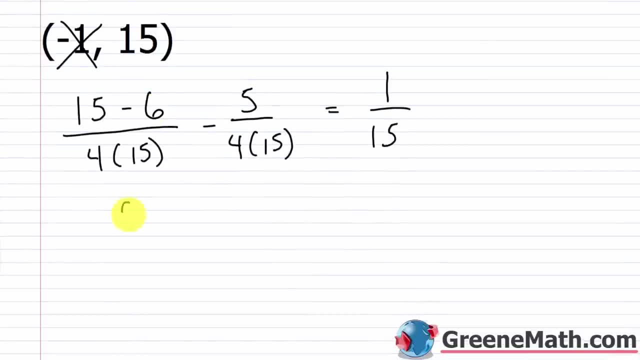 So 15 minus 6 in the numerator is 9. Over 4 times 15 in the denominator, that's 60. Then minus 5 over 4 times 15. Again, 4 times 15 is 60. 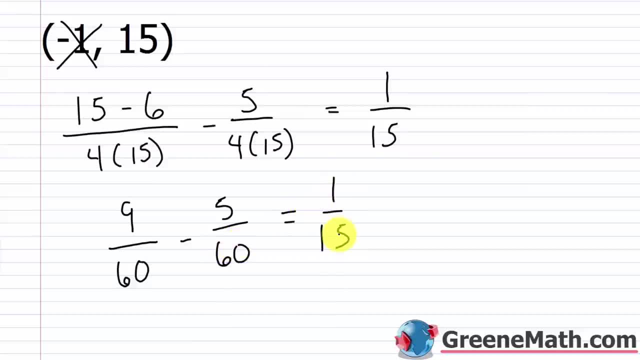 And this is equal to 1 over 15. So we have the same denominator here. What is 9 minus 5? That's 4. 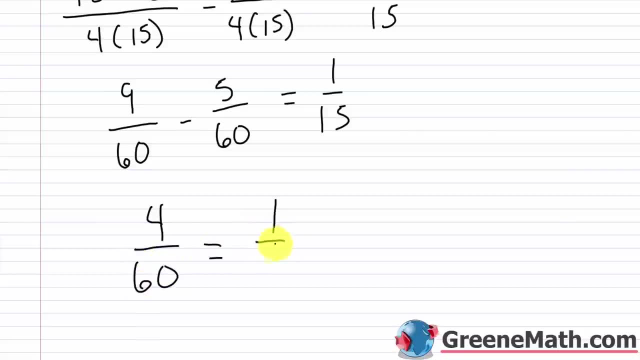 So we get 4 over 60 is equal to 1 15th. 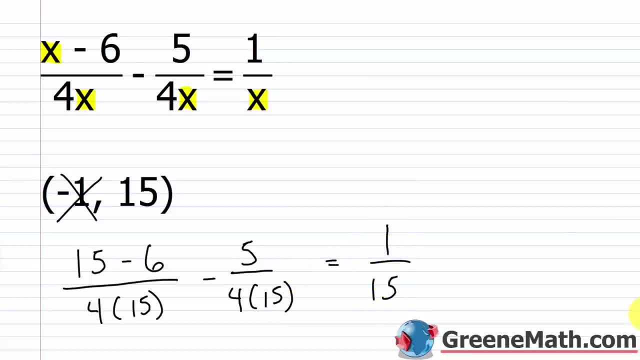 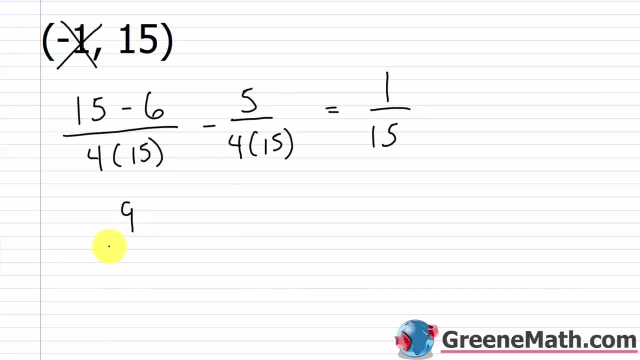 This should be equal to one over 15.. So let's crank this out real quick. So 15 minus six in the numerator is nine over four times 15. in the denominator that's 60. Then minus five over four times 15.. 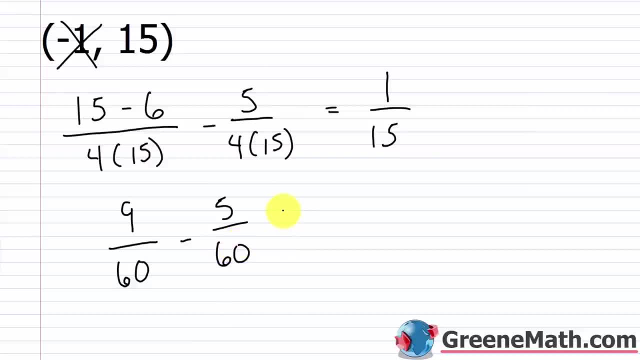 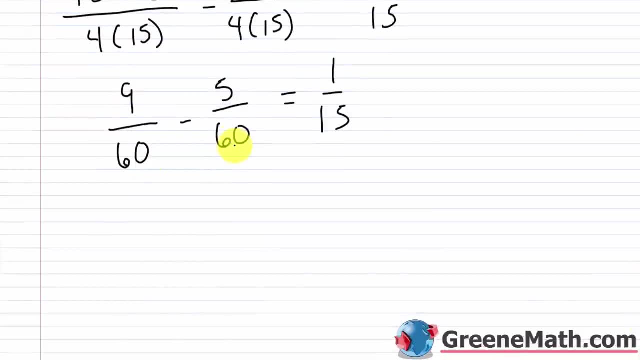 Again, four times 15 is 60. And this is equal to one over 15.. So we have the same denominator here. What is nine minus five? That's four. So we get four over 60 is equal to one 15th. 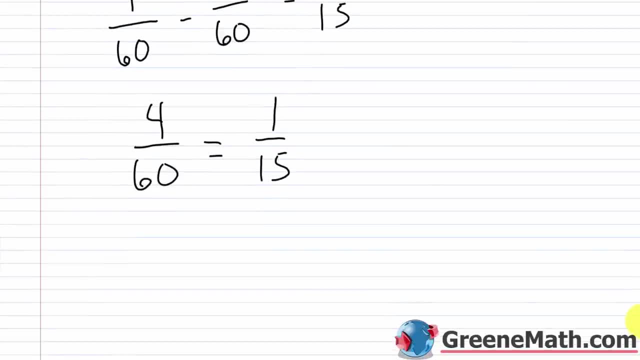 So at this point it doesn't seem like we have the same value on each side. but if we were to remember that we simplify our fractions, remember that 60 is divisible by four. 60 divided by four is 15.. So this I could cancel. 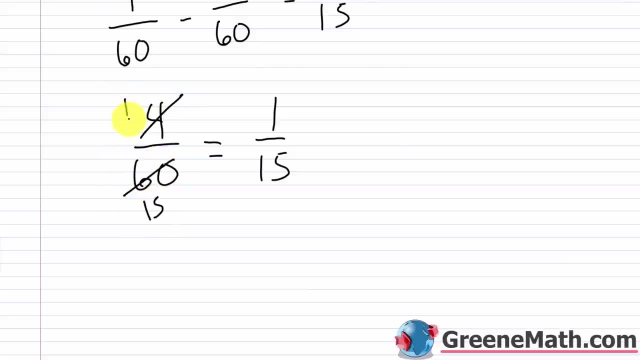 Cancel and make 15, cancel and make one. So really, what we'd end up with if we simplify, that is one 15th, So we have the same value on the left, on the right hand side, And so 15 is a solution for this equation. 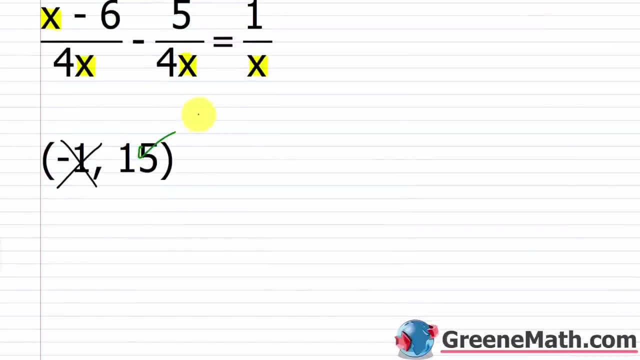 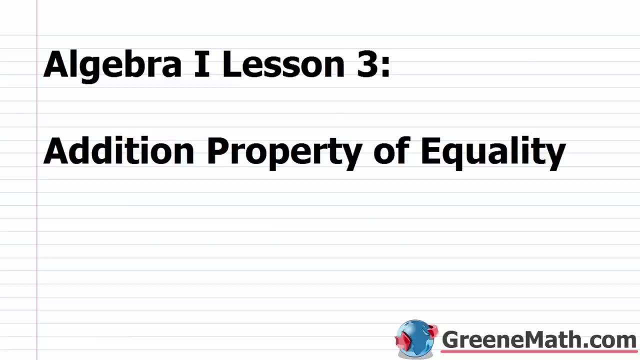 So we can go back up here and we can just put a check mark here: Yes, X equals 15 is a solution here. Hello and welcome to algebra one, lesson three. In this video we're gonna learn about the addition property of equality. 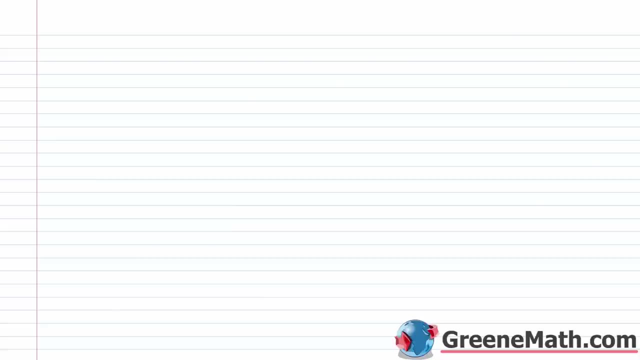 So in our first two lessons of our algebra one series, we learned some important vocabulary that's gonna help us throughout our course. The first thing we kind of talked about was that a variable is a symbol And generally it's a letter, a lowercase letter. 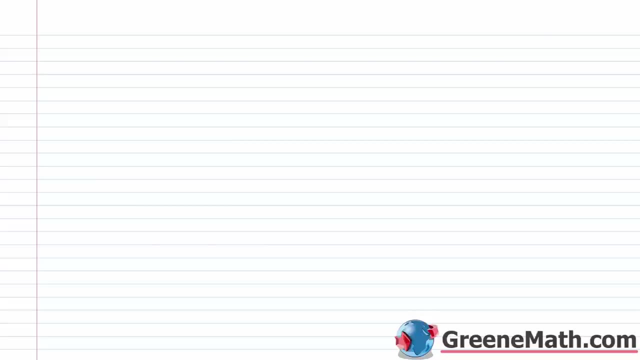 like X or Y or Z or any one that you wanna use, that represents some unknown value. Then we kind of moved on and we talked about something else known as a term. Now, a term is a single number, or it could also be a single variable. 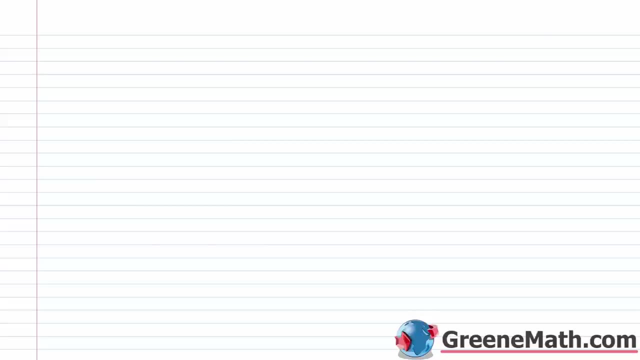 or it could be a number times one, or many variables, where your variables are possibly raised. two powers, So, as an example, a term could be again just a number, So let's say seven, or it could just be a variable, Let's say Y, or it could be a number. 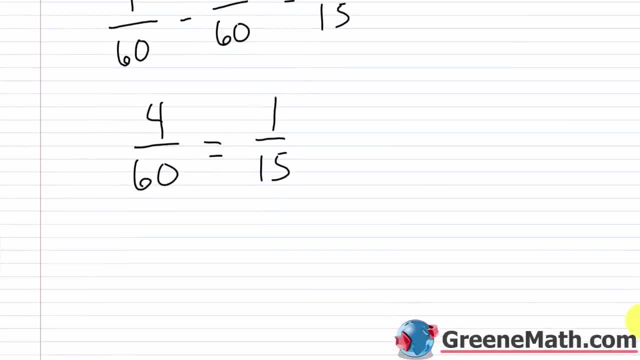 So at this point, it doesn't seem like we have the same value on each side. But if we were to remember that we simplify our fractions, remember that 60 is divisible by 4. 60 divided by 4 is 15. So this, I could cancel and make 15, cancel and make 1. So really, we're going to have 15 over 4 times 15. So what we'd end up with, if we simplify that, is 1 15th. So we have the same value on the left and the right-hand side. 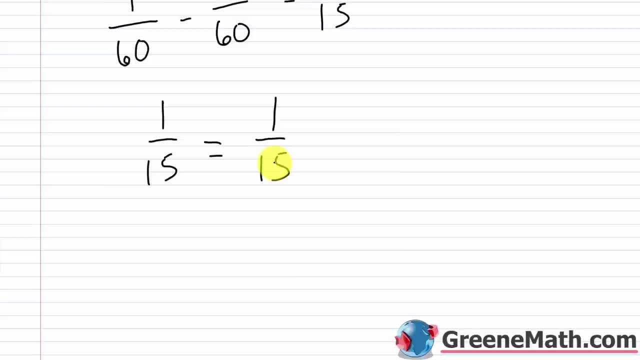 And so 15 is a solution for this equation. So we can go back up here, and we can just put a checkmark here. 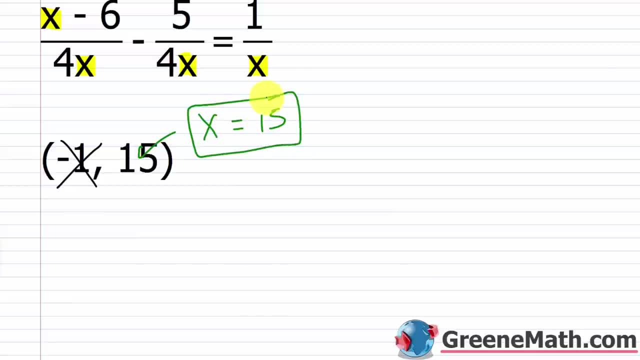 Yes, x equals 15 is a solution here. Hello, and welcome to Algebra 1, Lesson 3. 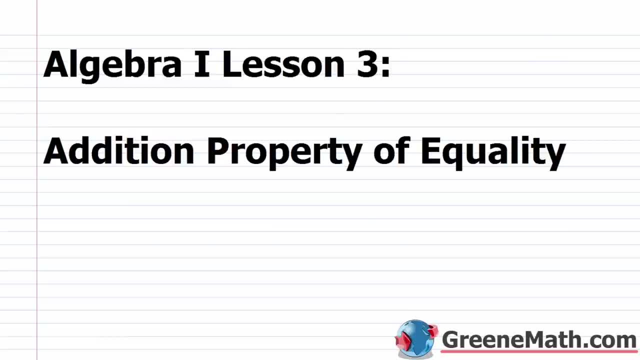 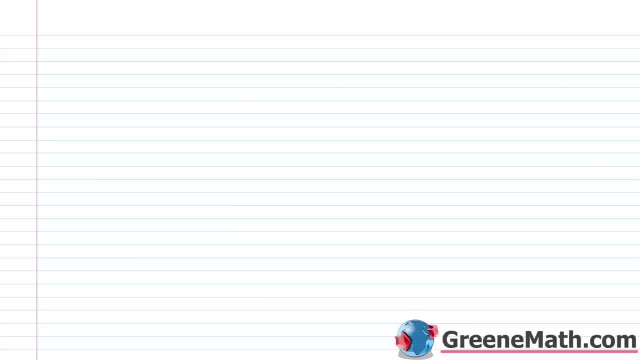 In this video, we're going to learn about the addition property of equality. So in our first two lessons of our Algebra 1 series, we learned some important vocabulary that's going to help us throughout our course. 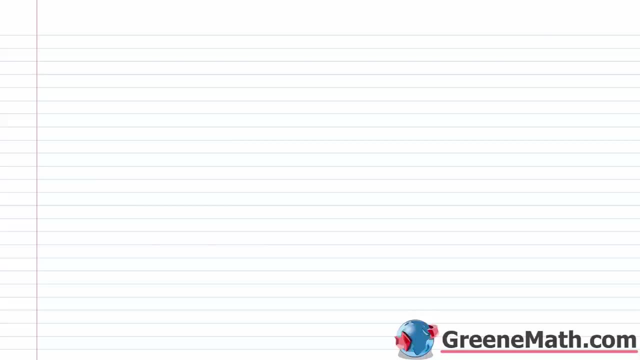 The first thing we kind of talked about was that a variable is a symbol, and generally it's a letter, a lowercase letter, like x or y or z or any one that you want to use that represents some unknown value. 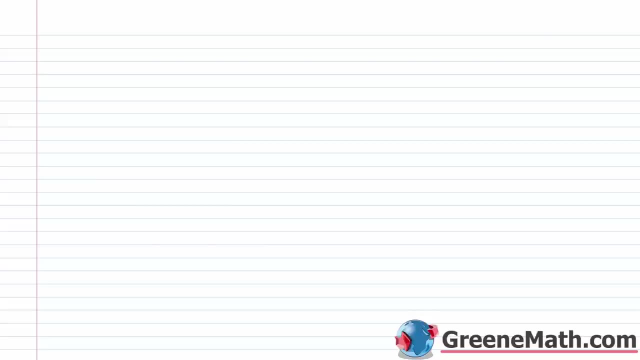 Then we kind of moved on, and we talked about something else known as a term. Now a term is a single number, or it could also be a single variable, or it could be a number times one or many variables where your variables are possibly raised two powers. So as an example, a term could be, again, just a number. So let's say 7, or it could just be a variable. Let's say y, or it could be a number times one or many variables. So I could have something like 7x, or I could have 2xy, or I could have 3x. 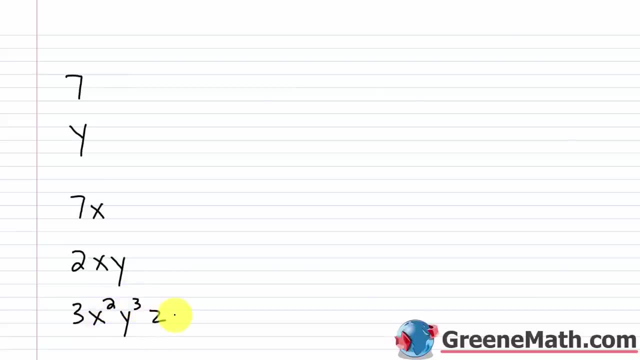 I could have x squared, y cubed, z, something like that. Each is an example of a term. 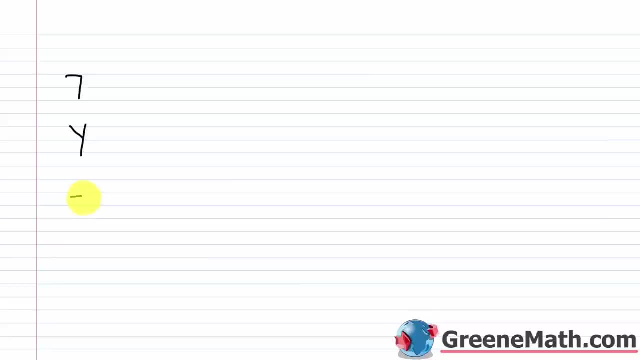 times one or many variables. So I could have something like seven X, or I could have two X, Y, or I can have three X squared Y, cubed Z, something like that. Each is an example of a term, Now kind of the next thing we talked about. 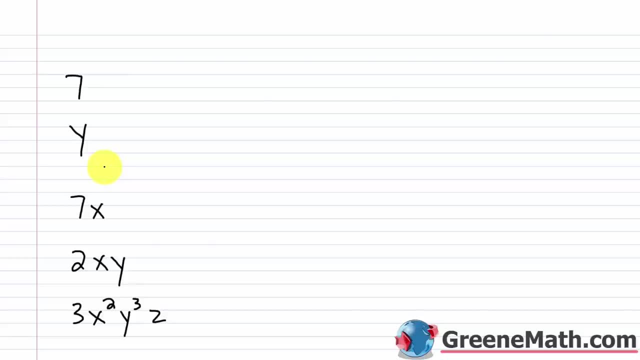 was an algebraic expression, So this is a single term. okay, so a single term by itself? or it's a collection of terms separated by plus or minus symbols. So, for example, let's say I had seven X minus two. So I have a term here and a term here. 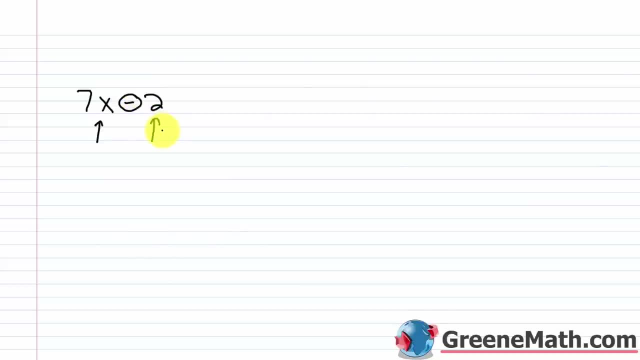 and it's separated by a minus symbol. So this is an algebraic expression, or I could just have a single term. I could just have the number three right. That's also an algebraic expression, or I could have something much more complex. 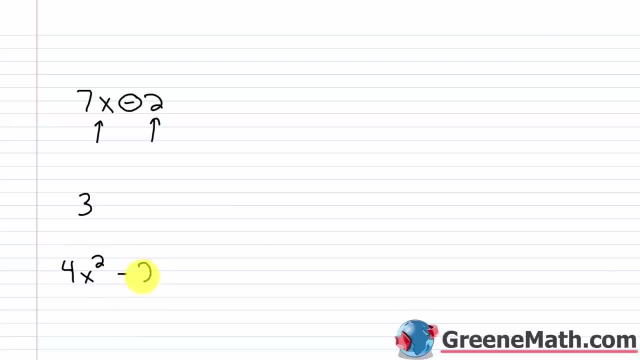 Let's say I had four X squared minus two Y plus 17.. Again, each term, okay, each term- is separated by the plus and minus signs. So this is a term: four X squared minus two Y plus 17.. Four X squared two Y is a term and 17 is a term. 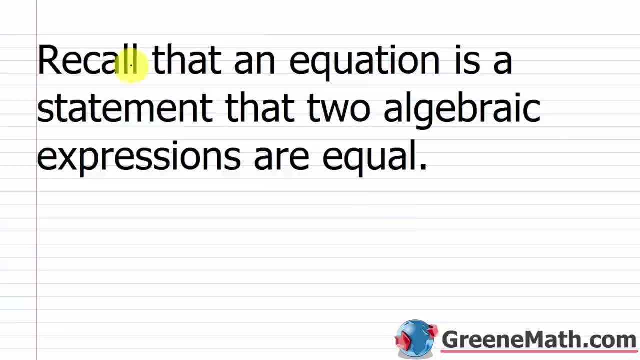 So then next, we kind of talked about equations. So I want you to recall that an equation is a statement that two algebraic expressions are equal. Now we fully understand what an algebraic expression is. at this point. Let's say I had something like two X plus three. 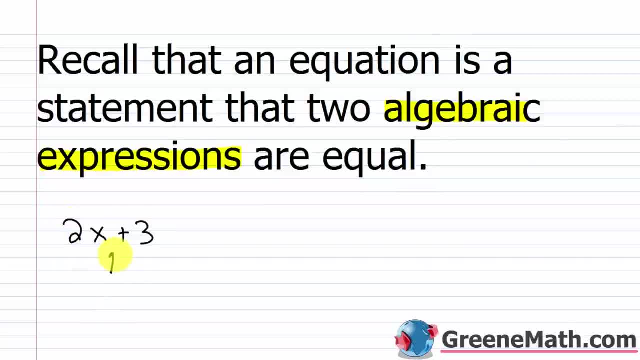 two X plus three. Again, we know that this is an algebraic expression. This is an algebraic expression. I have a term, two X- that's added to another term, That's three. right, That's following the definition of an algebraic expression. 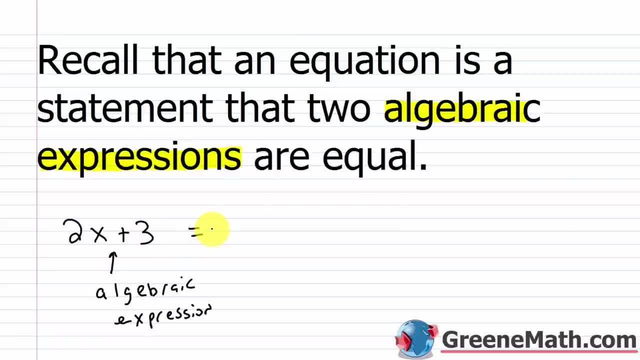 And let's say this is equal to another algebraic expression, just the number 11.. And again, this can also be an algebraic expression, because an algebraic expression again is a single term or it's a collection of terms separated by plus and minus. 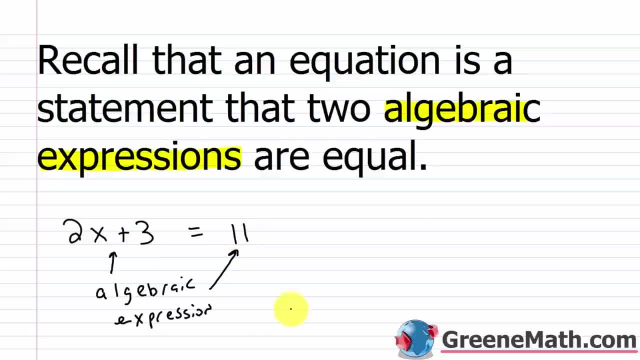 So we can have an algebraic expression or we can have an algebraic expression that has two plus or minus symbols. So in each case we have an algebraic expression, and now we've kind of thrown into the mix this equals sign. So what this tells me is that the left side is the same as 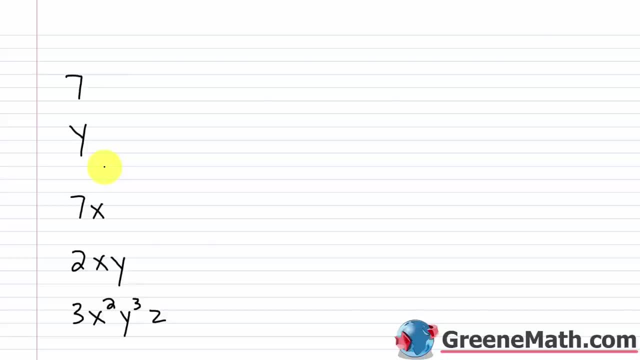 Now kind of the next thing we talked about was an algebraic expression. So this is a single term, okay, so a single term by itself, or it's a collection of terms separated by plus or minus symbols. So for example, let's say I had 7x minus 2. So I have a term here and a term here, and it's separated by a minus symbol. So this is an algebraic expression. 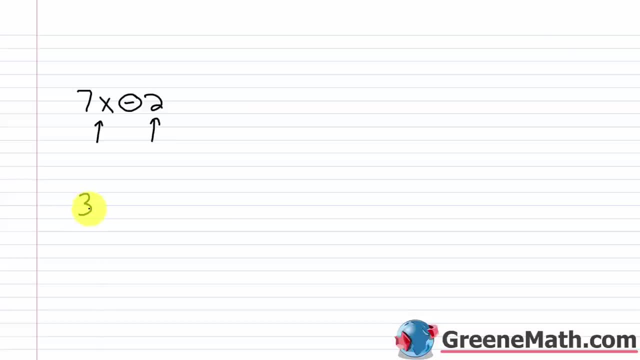 Or I could just have a single term. I could just have the number three, right? That's also an algebraic expression. 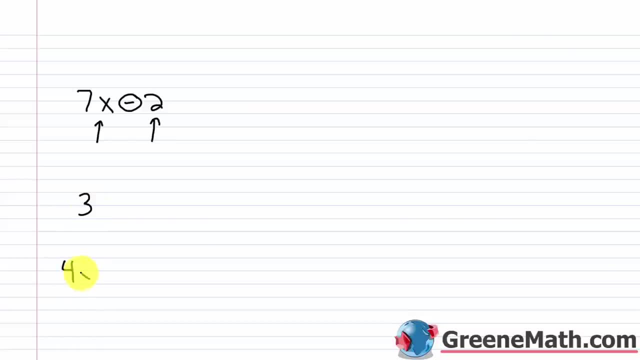 Or I could have something much more complex. Let's say I had 4x squared minus 2y plus 17. Again, each term, okay, each term is separated by the plus and minus signs. So this is a term, 4x squared, 2y is a term, and 17 is a term. So then next we kind of talk about the algebraic expression. So we talked about equations. 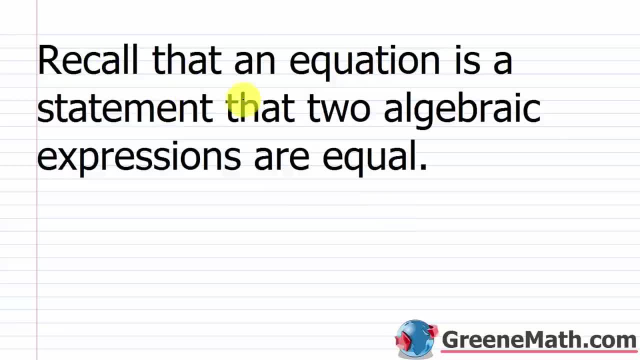 So I want you to recall that an equation is a statement that two algebraic expressions are equal. 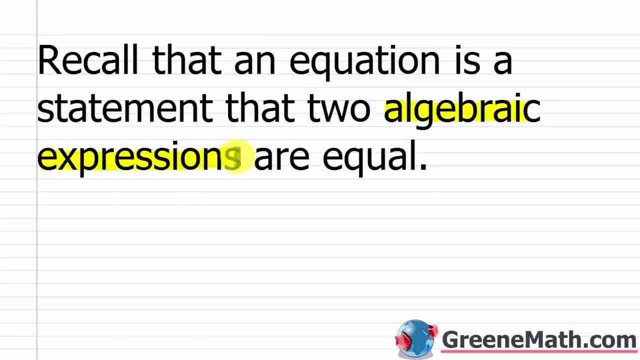 Now we fully understand what an algebraic expression is at this point. Let's say I had something like 2x plus 3, 2x plus 3. 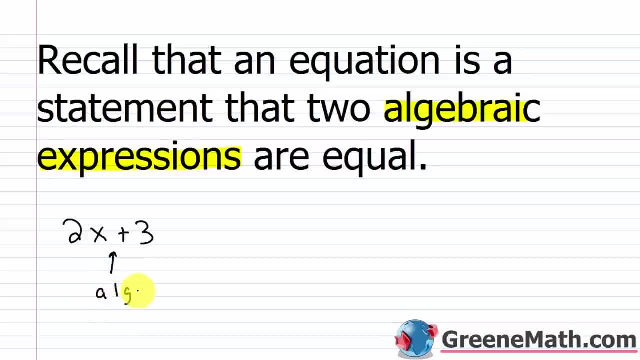 Again, we know that this is an algebraic expression. This is an algebraic expression, right? I have a term 2x. That's added to another term. That's 3, right? That's following the definition of an algebraic expression. 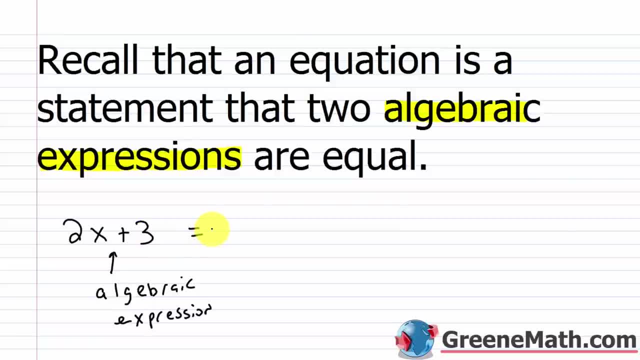 And let's say this is equal to another algebraic expression, just the number 11. And again, this can also be an algebraic expression because an algebraic expression, again, is a single term or it's a collection of terms separated by plus or minus symbols. 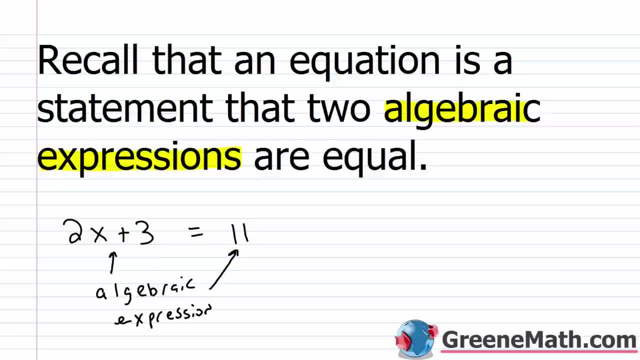 So in each case, we have an algebraic expression. And now we've kind of thrown in, you know, into the mix this equals sign. 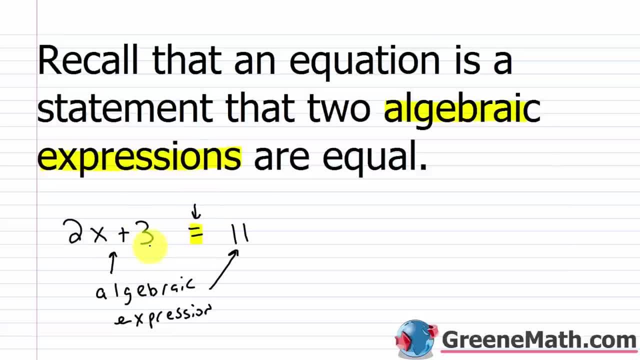 So what this tells me is that the left side is the same as or is equal to the right side. 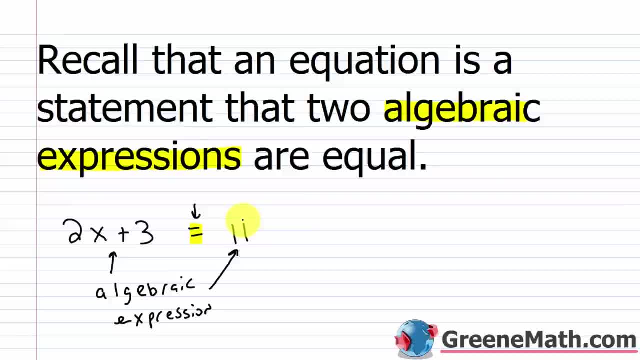 You can kind of think of some definitions of things being equal in your life. If we have equal pay, that means we make the same amount. 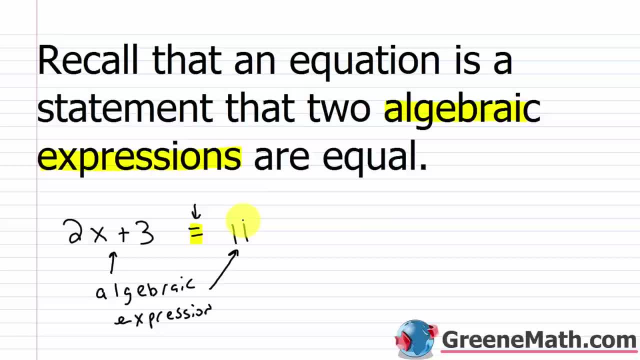 or is equal to the right side. You can kind of think of some definitions of things being equal in your life. If we have equal pay, that means we make the same amount, And so our ultimate goal when we're solving an equation- 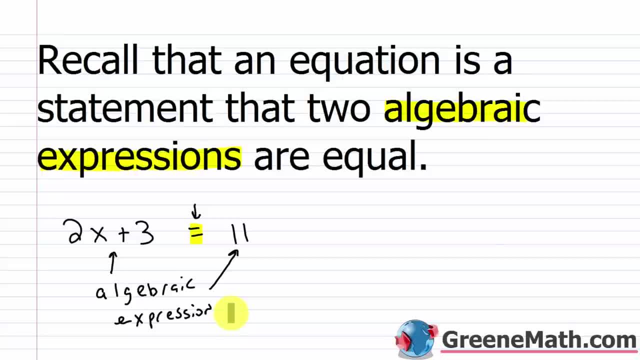 or in some cases the values that when substituted in for the variable, or in some cases you'd have variables- that makes the equation true. It means making the equation to where the left side and the right side are the exact same value. And again, let me kind of further clarify this. I'm telling 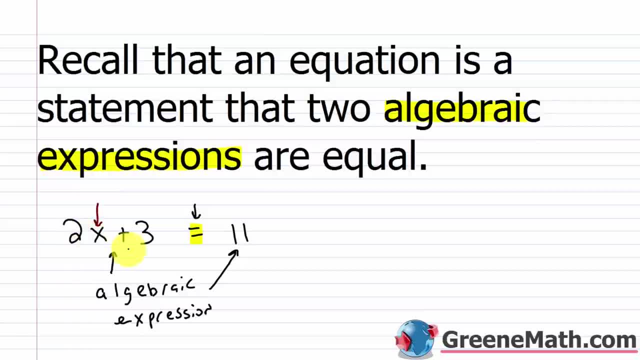 you that you can plug something in for x and simplify over here, and the left side would also be 11, right, At this point, 2x plus 3 doesn't look like it's the same thing as 11.. But if I plug in, 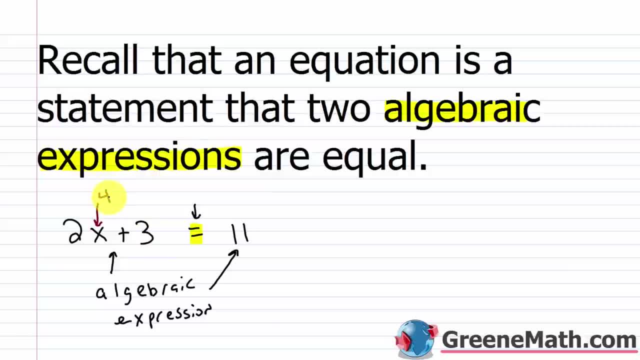 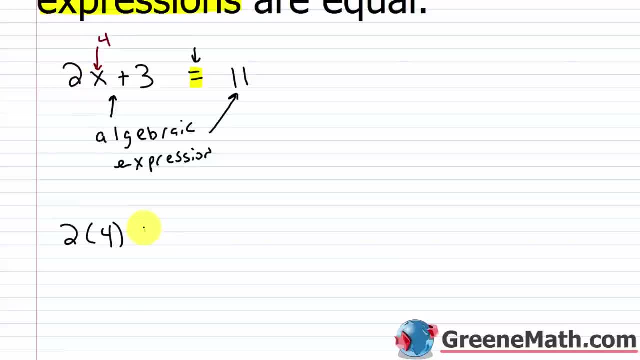 the number 4 for x. let's see what happens On the left. I would have 2 times 4.. Again, all I did was I replaced the variable x with 4, plus 3 equals 11.. So 2 times 4 would be done first, because of. 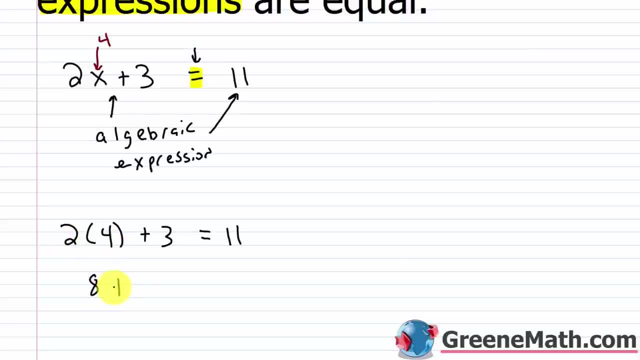 our order of operations: 2 times 4 is 8, so we'd have: 8 plus 3 equals 11.. And then on the left side, 8 plus 3 equals 11.. So 2 times 4 is 8, so we'd have: 8 plus 3 equals 11.. And then on the left side: 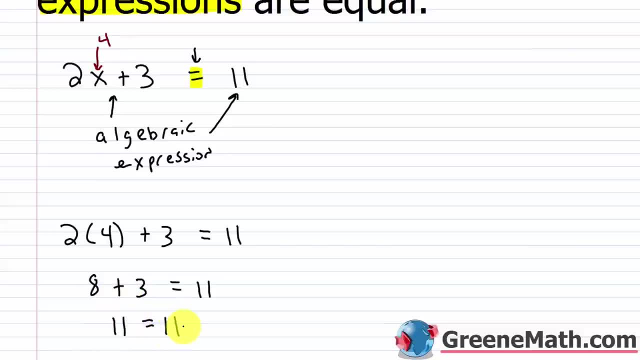 3 is 11.. So 11 equals 11.. So when I replace my variable x with the number 4, what happens is, through simplification, I end up with the same exact value on the left as the right, And so our 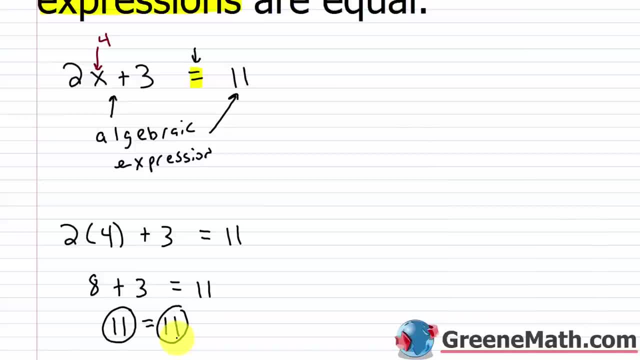 equation we'd say is true now because the same value occurs on the left and the right, We can say we have a true statement. Now, 4 is the only value that happens to give me a true statement. If I replace x with anything else, it would be false. So let me show you an example. Let's say 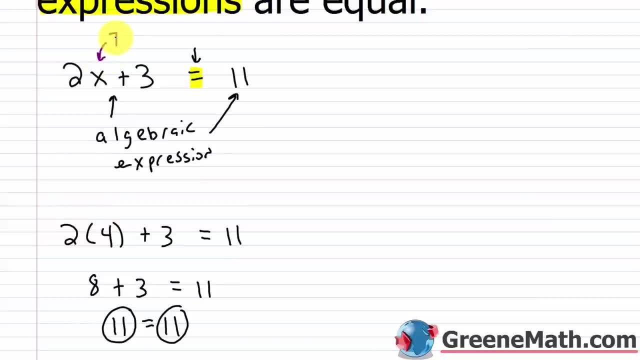 that I said: okay, I think x is equal to 7. And I plug in a 7 for x. What's going to happen here? Well, you probably can guess that I'm not going to have the same value on the left and the right. 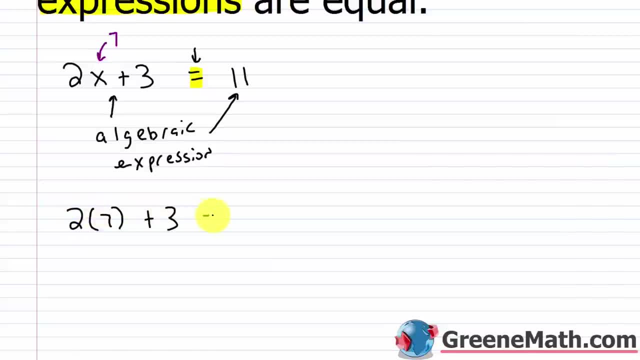 2 times 7 would be done. now plus 3 equals 11.. 2 times 7 is 14.. 14 plus 3 equals 11.. 14 plus 3 is 7. 17.. 17 is not equal to 11.. 17 is not the same value as 11, right, They're not equal, If I made. 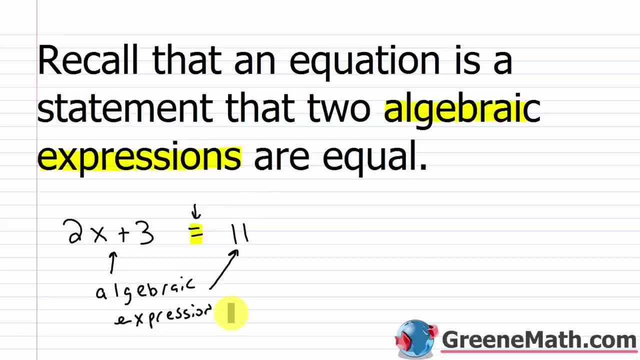 And so our ultimate goal when we're solving an equation is to find the value or in some cases the values that when substituted in for the variable or in some cases, you can call it the value of the equation, you would have variables, that makes the equation true. It means making the equation to where the left side and the right side are the exact same value. 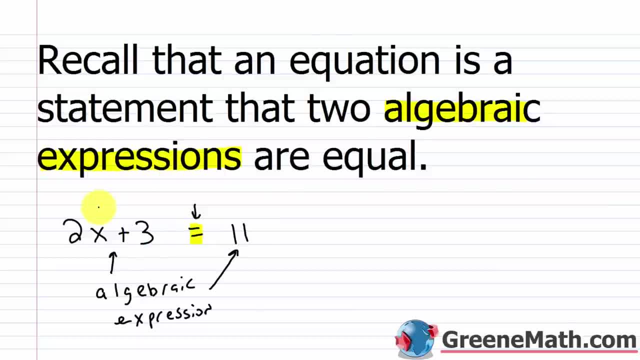 And again, let me kind of further clarify this. I'm telling you that you can plug something in for x and simplify over here and the left side would also be 11, right? 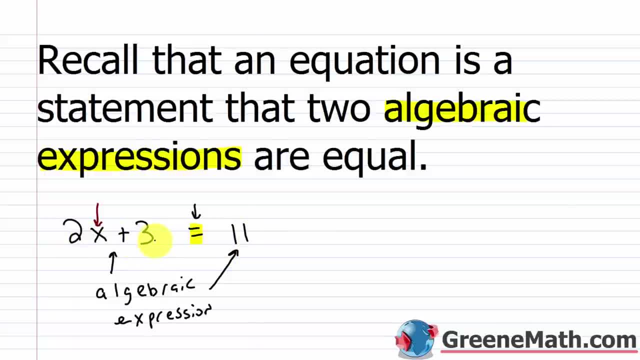 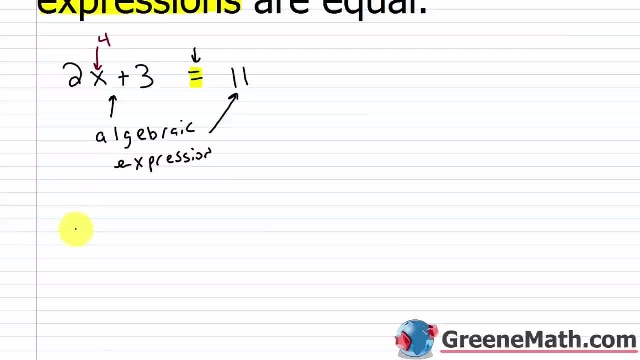 At this point, 2x plus 3 doesn't look like it's the same thing as 11. But if I plug in the number 4 for x, let's see what happens. On the left, I would have 2 times 4. Again, all I did was I replaced the variable x with 4 plus 3 equals 11. So 2 times 4 would be done first because of our order of operations. 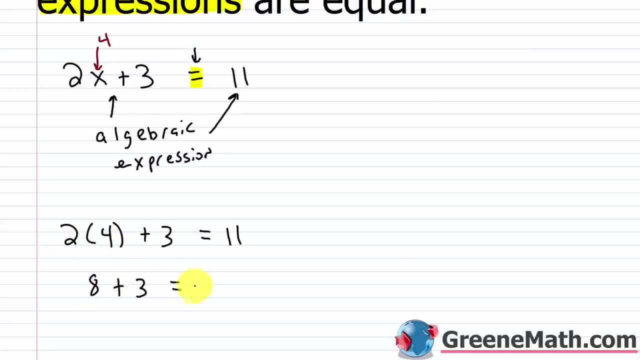 2 times 4 is 8, so we'd have 8 plus 3 equals 11. And then on the left side, 8 plus 3 is 11, so 11 equals 11. 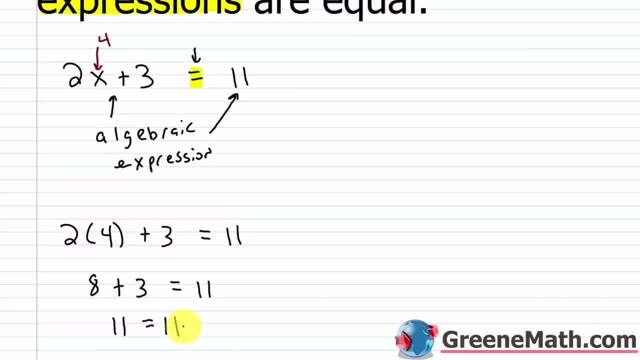 So when I replace my variable x with the number 4, what happens is through simplification, I end up with the same exact value on the left as the right. 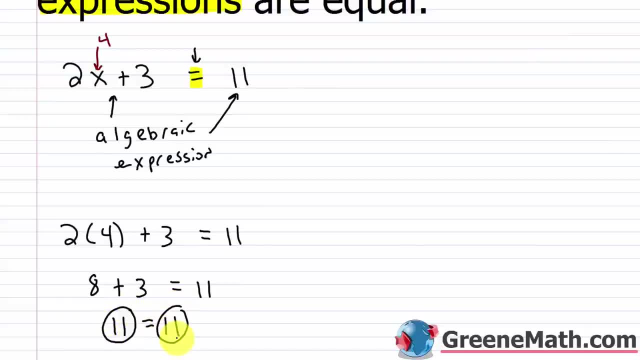 And so our equation, we'd say, is true now because the same value occurs on the left and the right. We can say we have a true statement. Now, 4 is the only value that happens to give me a true statement. 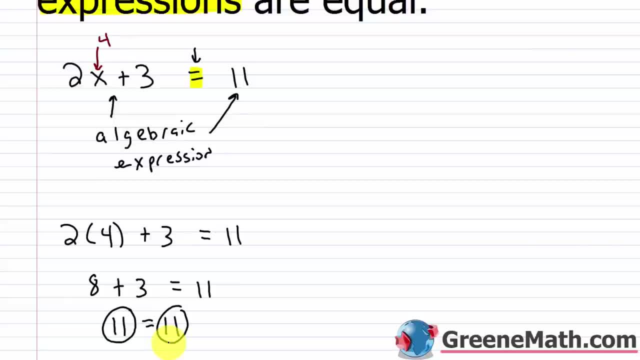 If I replace x with anything else, it would be false. So let me show you an example. 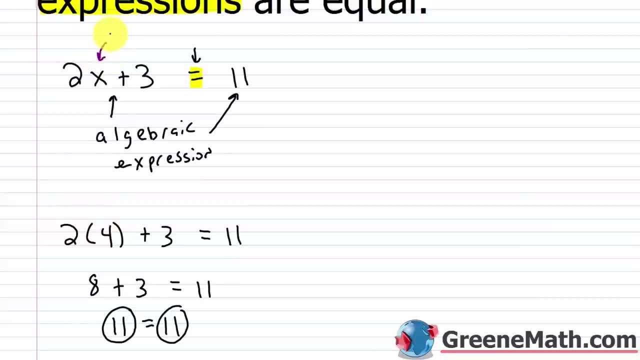 Let's say that I said, okay, I think x is equal to 7. And I plug in a 7 for x. What's going to happen here? 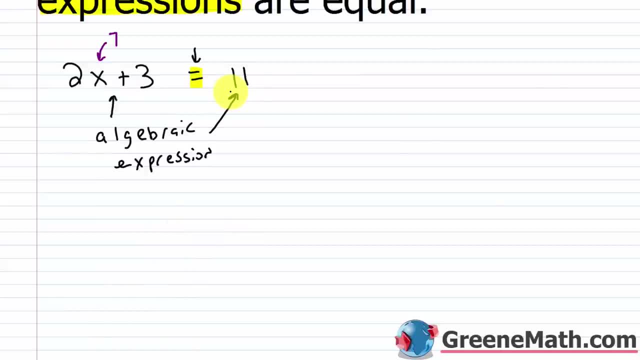 Well, you probably can guess that I'm not going to have the same value on the left and the right. 2 times 7 would be done now, plus 3 equals 11. 2 times 7 is 14. 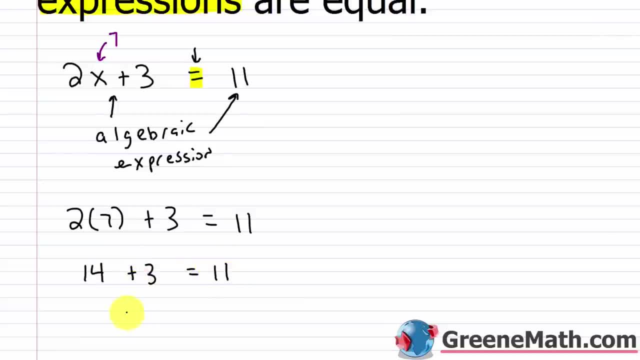 14 plus 3 equals 11. 14 plus 3 is 17. 17 is not equal to 11. 17 is not the same value as 11. They're not equal. 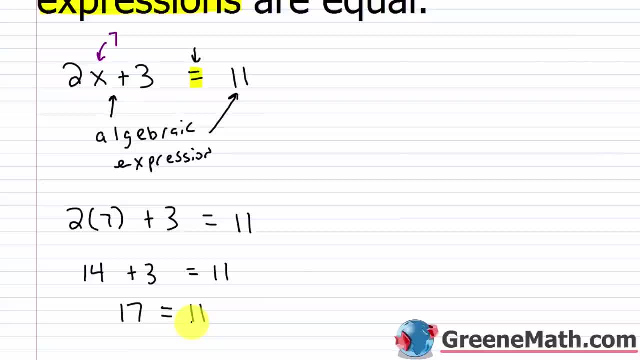 If I made $17 and you made $11, we don't have equal pay. So at this point, we can say that this is false. 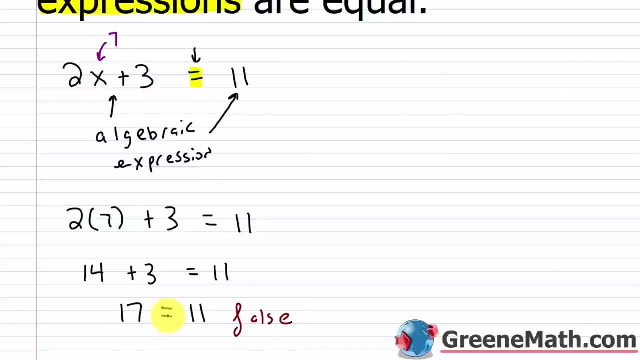 This is a false statement because 17 does not equal 11. 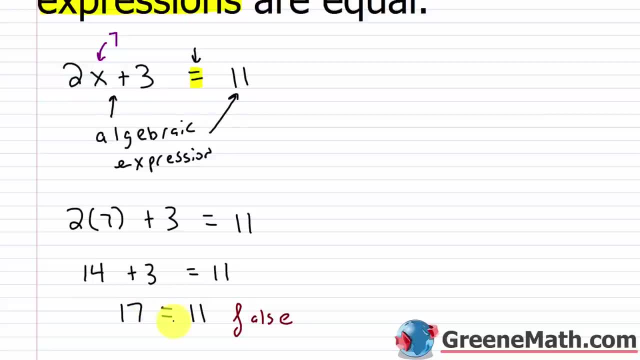 And right here, I'm saying that they are equal. So it's kind of a contradiction. 17 is not equal to 11, so we say it's a false statement. 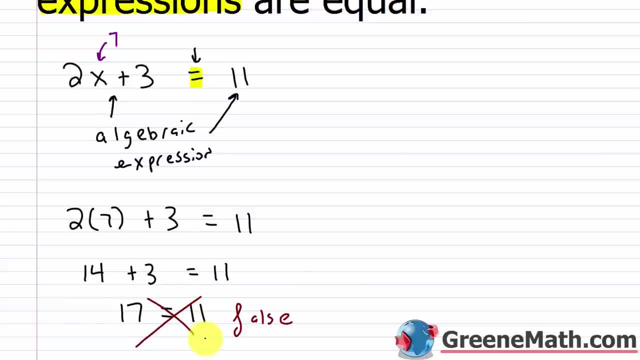 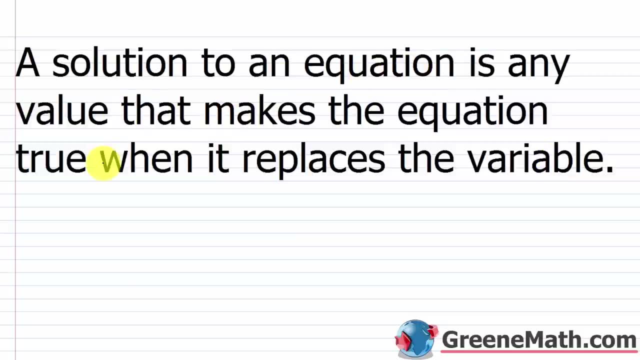 So again, only x equals 4 is a solution to this equation. So again, officially, if you want to write this down in your notes, a solution to an equation is any value that makes the equation true when it replaces the variable. 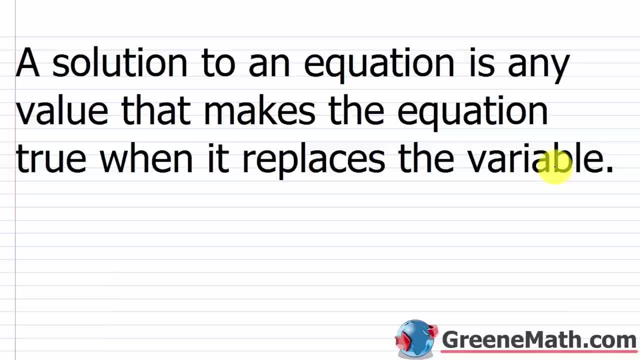 So in the last example, we saw that if we replaced the variable with 4, we got a true statement. 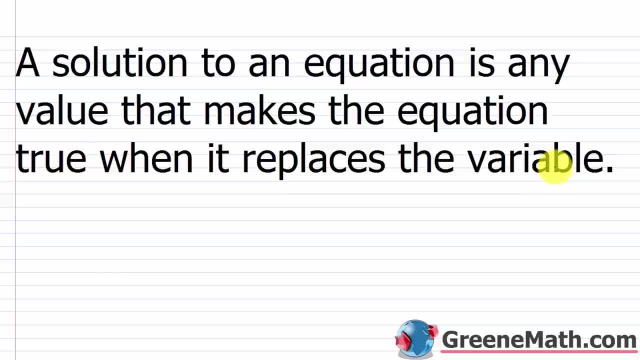 The left and the right side were both 11. If we replace the variable with anything else, we won't get the same number on each side. And so it's not a solution. All right. 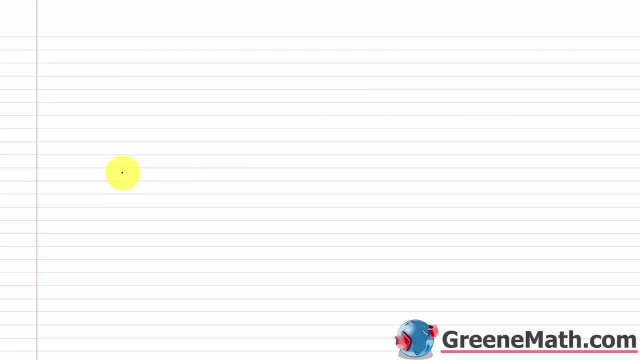 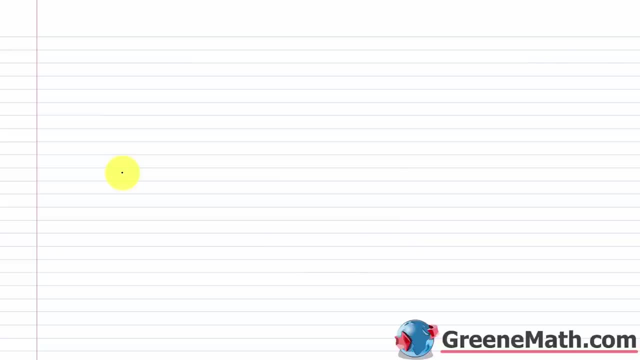 Well, what we're going to focus on right now, we're going to focus on very, very simple equations. So the first chapter in your textbook on solving equations is going to be dedicated to solving linear equations. 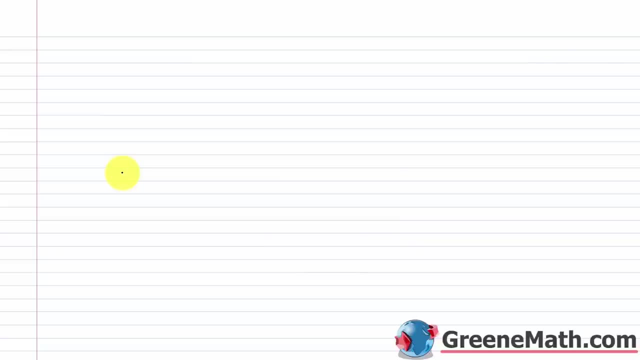 And it's going to be linear equations in one variable. So one variable is involved. And they look like this. So you might see this in your textbook. 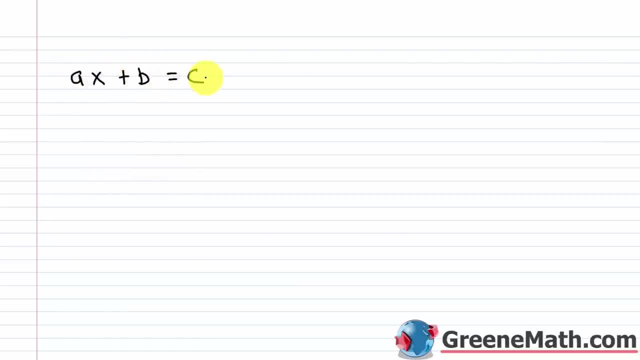 Ax plus b equals c. And x is our variable. But really, you can use anything. I could write this as ay plus b equals c. Or I could write az plus b equals c. You can use anything as your variable. It doesn't matter. 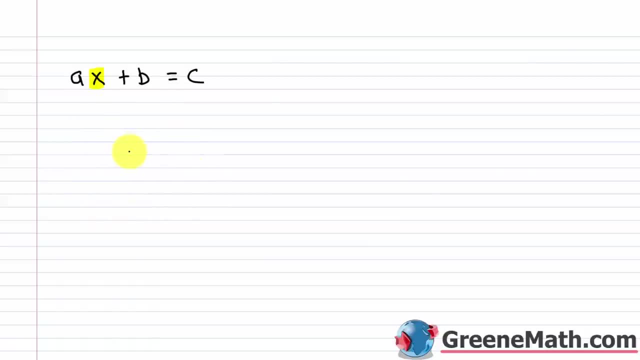 But typically, we use x. So that's why this is presented like this in your textbook. And I want to talk a little bit about kind of some 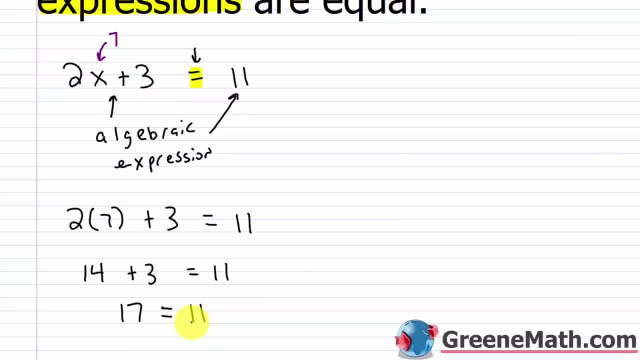 $17 and you made $11, we don't have equal pay. So at this point we can say that this is false. Right, This is a false statement, because 17 does not equal 11.. And right here I'm saying that. 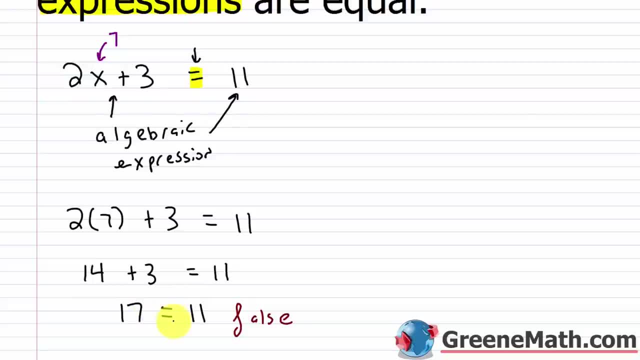 they are equal. So it's kind of a contradiction. right 17 is not equal to 11.. So we say it's a false statement. So again, only x equals 4 is a solution to this equation. So again, officially. 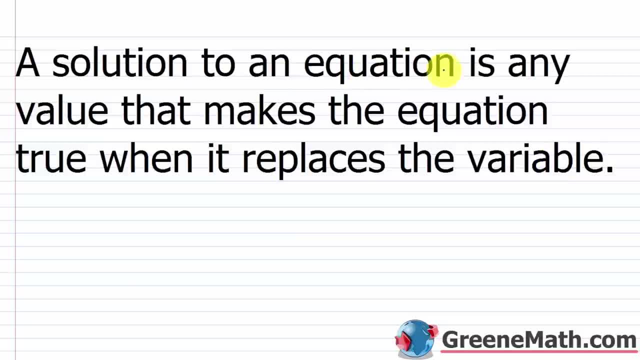 if you want to write this down in your notes. a solution to an equation is any value that makes the equation true when it replaces the variable. So in the last example we saw that if we replace the variable with 4, we got a true statement. The left and the right side were both 11.. 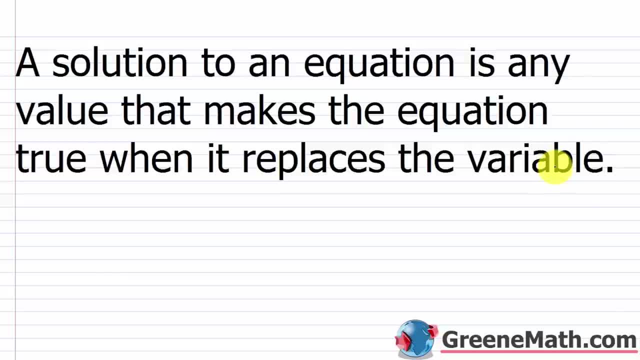 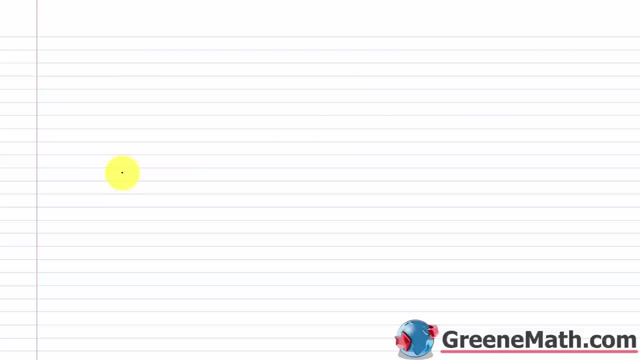 If we replace the variable with anything else, we won't get the same number on each side, And so it's not equal to 11.. So again, only x equals 4 is a solution to this equation, Not a solution, All right? So so far, up to this point, I've been giving you solutions to our 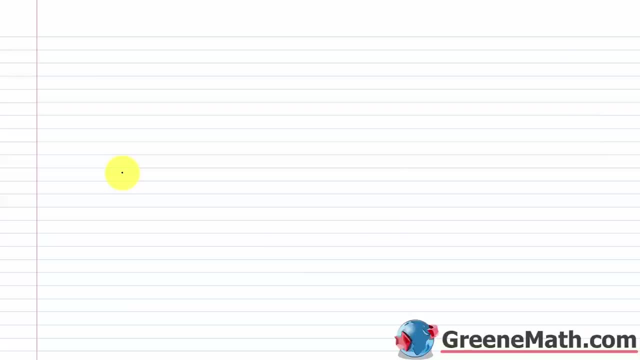 equations that we're working with And we've kind of just plugged in and we've seen if it works or if it doesn't work, But how do you actually go about getting the solution? Well, what we're going to focus on right now we're going to focus on very, very simple equations. So the first: 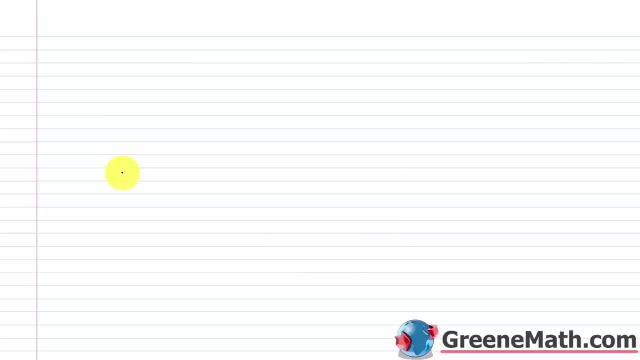 chapter in your textbook on solving equations is going to be dedicated to solving linear equations And it's going to be linear equations in one variable, So one variable is involved, And they look like this, So you might see this in your textbook: ax plus b equals c, And x is our. 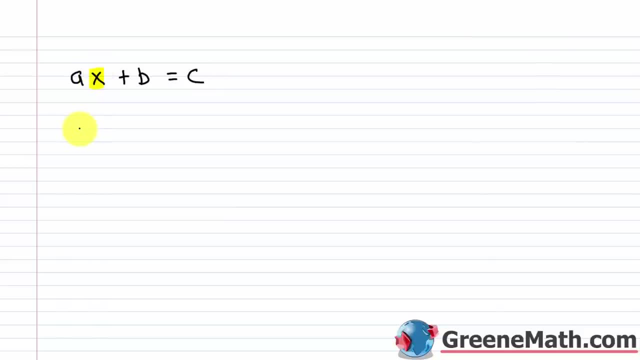 variable, But really you can use anything. I could write this as: ay plus b equals c. or I could write az plus b equals c. You can use anything as your variable, It doesn't matter. But typically we use x. So that's why this is present And we're going to use x as our variable And we're going to 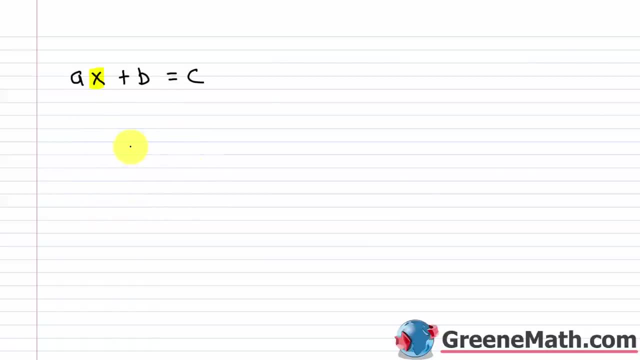 it like this in your textbook, And I want to talk a little bit about, kind of some of these letters that we're using here: a, b and c. The first thing is that they can be any real numbers- And we haven't really defined what a real number is- But just kind of anything you can think about at this. 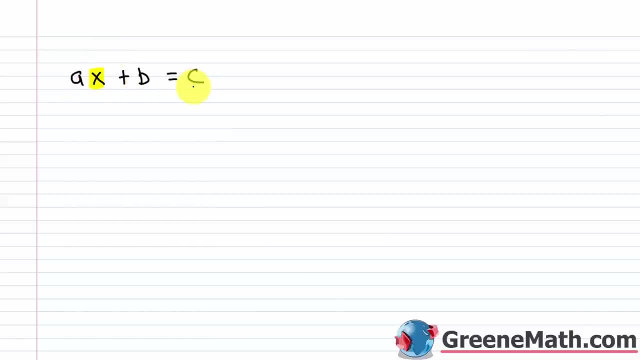 of these letters that we're using here, a, b, and c. The first thing is that they can be any real numbers. And we haven't really defined what a real number is. But just kind of anything you can think about at this point. 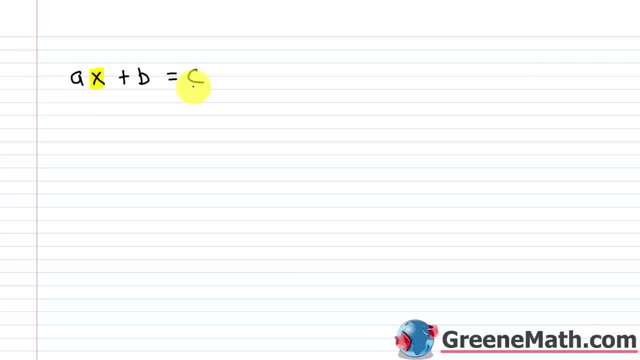 Fractions, decimals, negatives, integers, anything you've worked with can be plugged in for a, b, or c with one restriction. We cannot have a equal to 0. And the reason for that is if I plug a 0 in for a, I would have 0 times x. And 0 times anything is 0. So if I plugged in a 0 for a, 0 times x is 0, that's gone. And so I don't have a variable anymore. 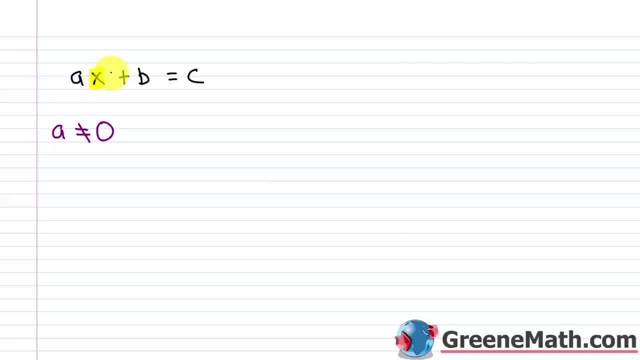 I just have b equals c. And that's only true if b and c are the same number. 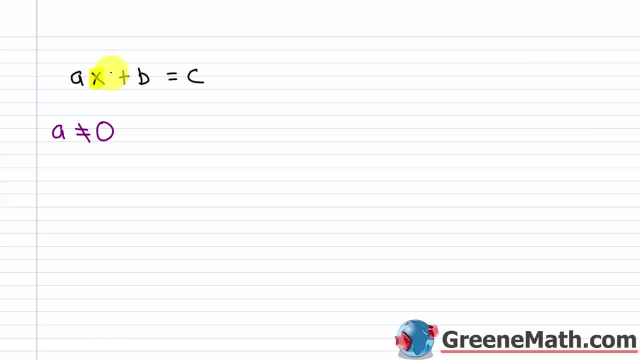 So a, b, and c can be any real number. Only a can't be 0. Now, b could be 0. c could be 0. That restriction is just on a. 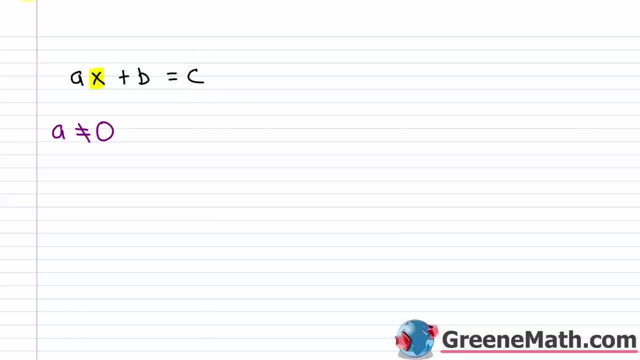 Let's talk a little bit about what a is called. 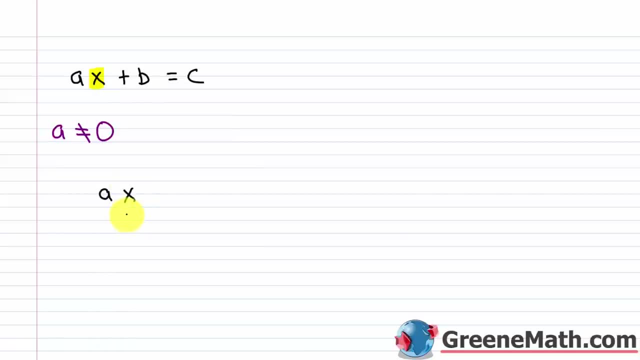 So a is the number that is multiplying your variable. When a number is multiplying a variable, it's called a coefficient. 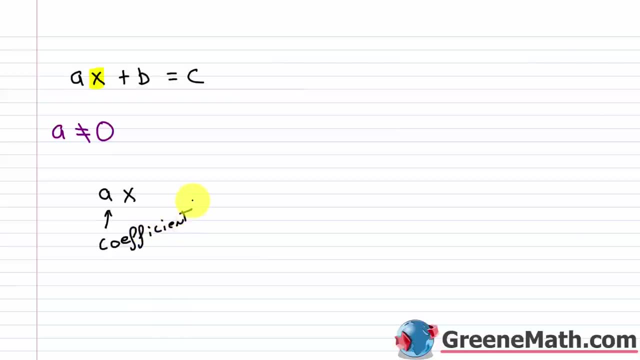 And that's very important to write that down or memorize it in some way, because that's going to come up a lot. 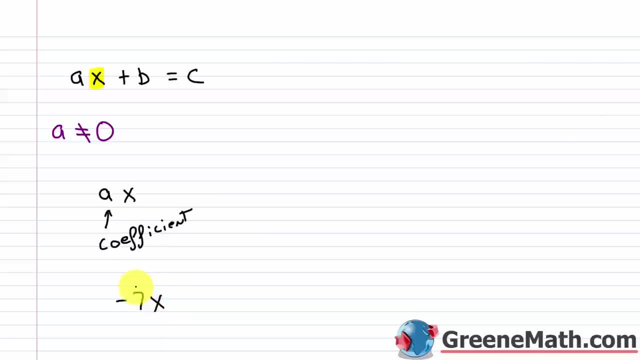 So if I had something like negative 7x, we say that negative 7, the number that's multiplying x, is the coefficient of x. 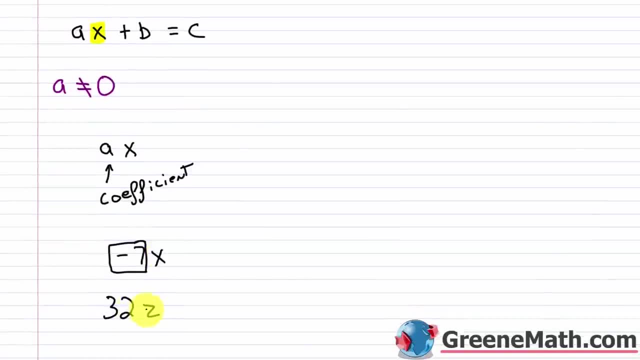 Or if I had, let's say, 32z, 32 is multiplying the variable z. So 32 is the coefficient of z. 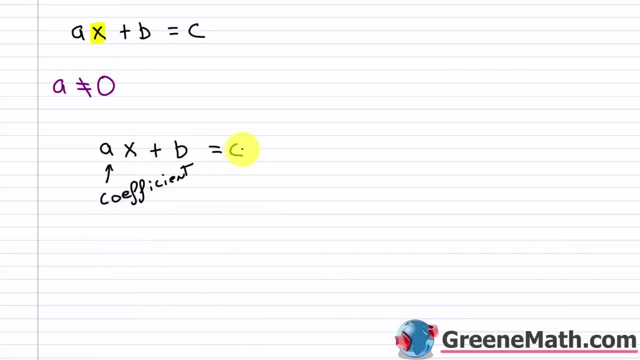 Now, then we have plus b equals c. Now, there's no variable. It's just the number that's multiplying the variable z. 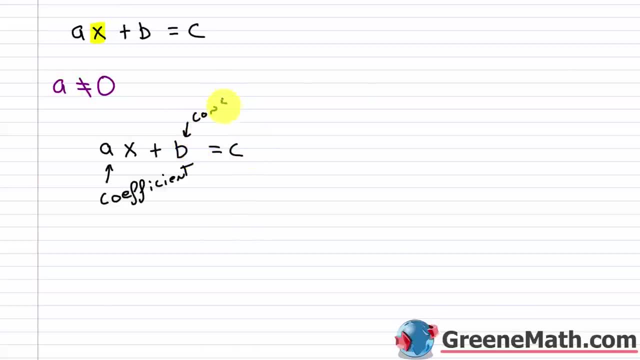 So if I had something like negative 3x minus 7 equals 2, this negative 7 and this 2, those are both constants. 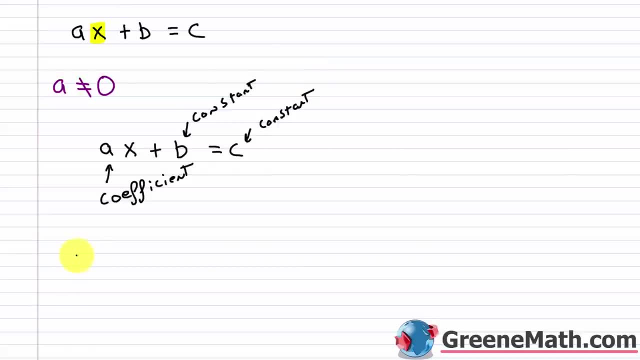 And then this negative 3 here, the number that's multiplying the variable z, is the coefficient of x. 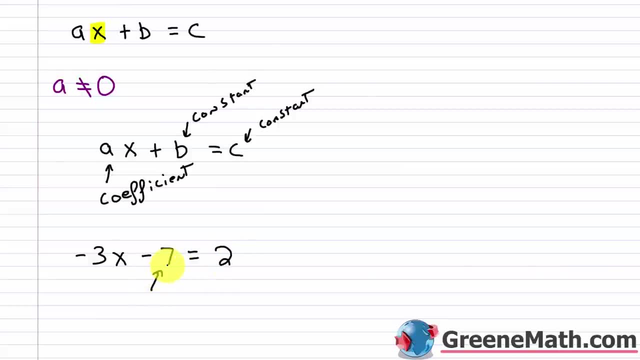 So that's the constant. So if I had something like negative 3x minus 7 equals 2, 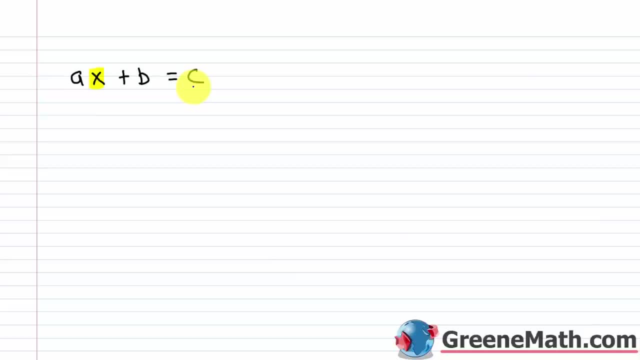 point. fractions, decimals, negatives, you know integers, anything you've worked with can be plugged in for a, b or c, with one restriction: We cannot have a equal to 0.. And the reason for that: plug a zero in for a, I would have zero times x and zero times anything is zero. So if I plugged 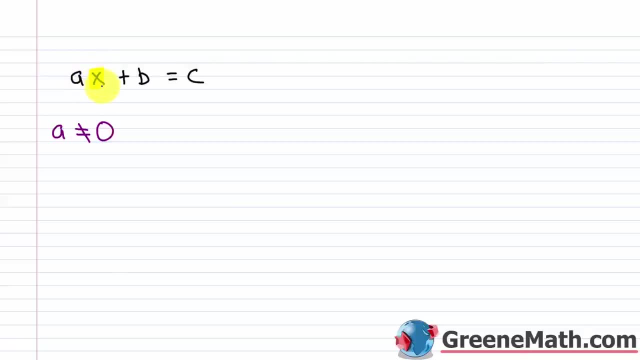 in a zero, for a zero times x is zero. that's gone, and so I don't have a variable anymore, right? I just have b equals c, and that's only true if b and c are the same number, right? So 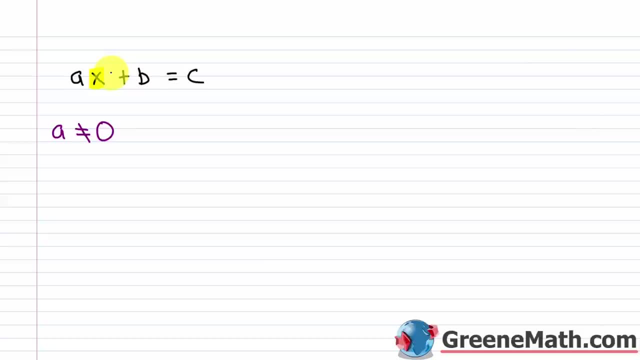 that doesn't work for us. So a, b and c can be any real number. only a can't be zero. Now, b could be zero, c could be zero. okay, That restriction is just on a. Let's talk a little. 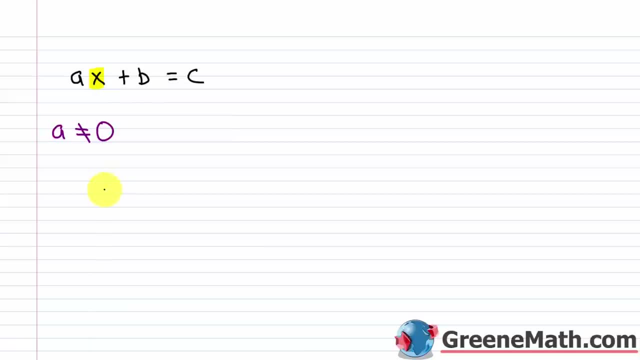 bit about what a is called. So a is the number that is multiplying your variable. When a number is multiplying a variable, it's called a coefficient. a coefficient And that's very important to write that down or memorize it in some way, because that's going to come up a lot. 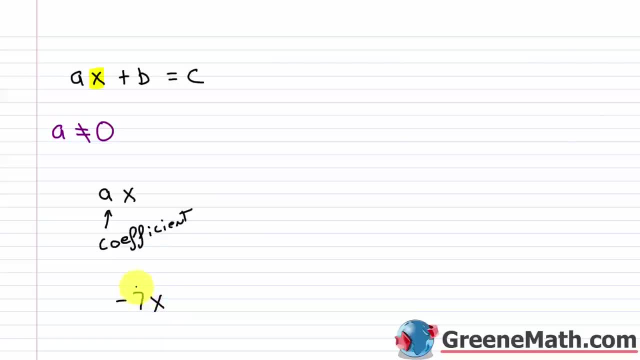 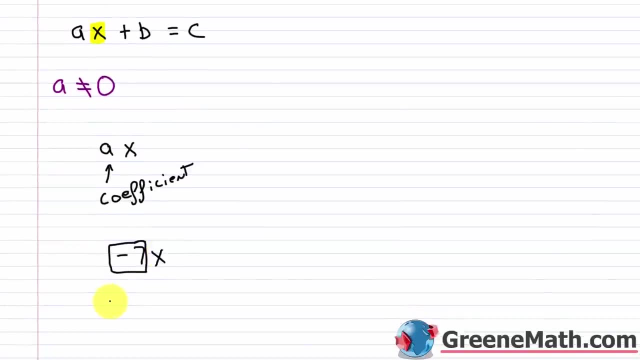 So if I had something like negative 7x, we say that negative 7, the number that's multiplying x is the coefficient of x. Or if I had, let's say, 32z, 32 is multiplying the variable z, so 32 is the coefficient of z. 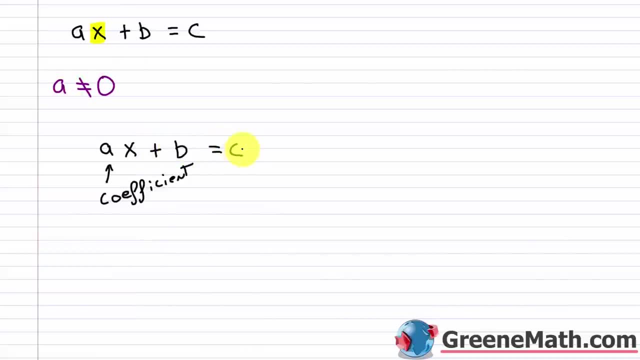 Now then we have plus b equals c. Now there's no variable involved in b or c, so when that happens, we call these constants. So this is a constant and this is called a constant, okay, So this is just kind of a number hanging out by itself. So 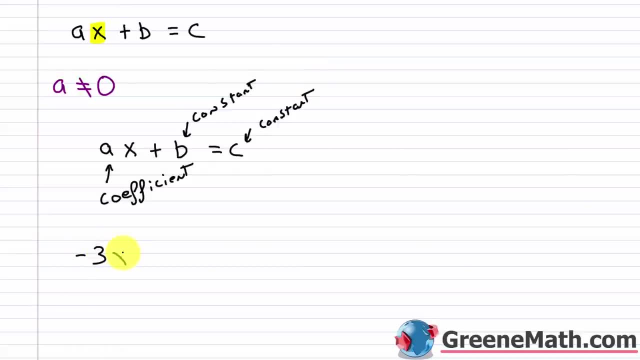 For example, if I had something like negative 3x minus 7 equals 2, this negative 7 and this 2, those are both constants. And then this negative 3, here the number that's multiplying x, that's a coefficient right. 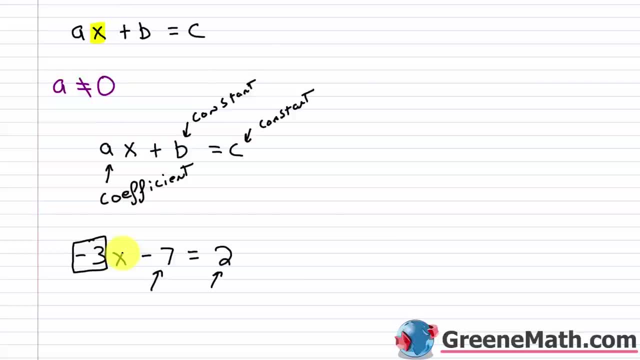 That's the coefficient of x. All right, so today we're going to kind of start off. let me kind of erase this. I'm going to show you what we're going to be working through, and then we're going to jump right in. 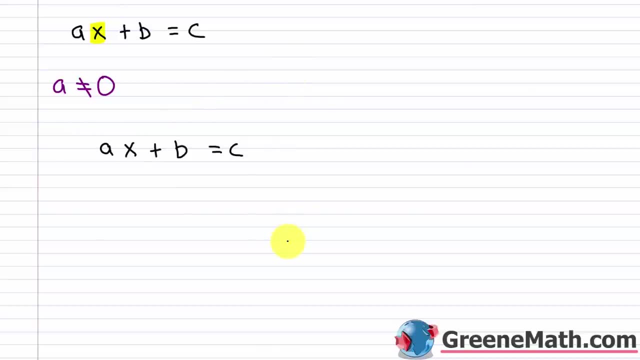 All right. so we're going to start off with a very simple type of linear equation. one variable It's where a equals 1, so a is 1, so you would have 1x and 1 times. something is just itself. 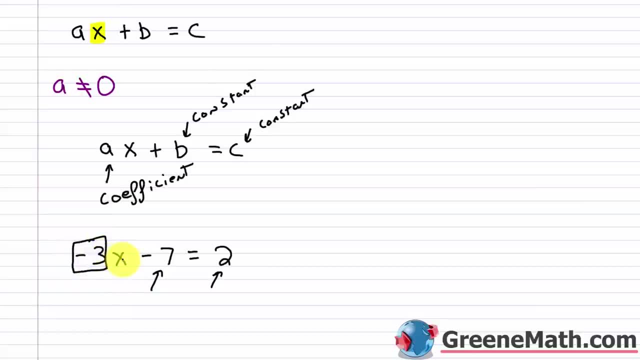 this negative 7 and this 2, those are both constants. And then this negative 3 here, the number that's multiplying x, that's a coefficient. That's the coefficient of x. All right. So today, we're going to start off. Let me erase this. 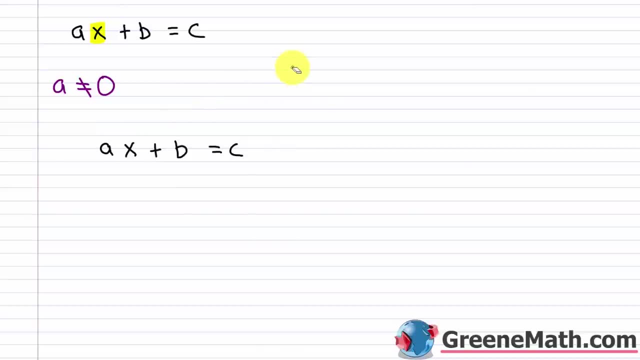 I'm going to show you what we're going to be working through. And then we're going to jump right in. So we're going to start off with a very simple type of linear equation of one variable. It's where a equals 1. So a is 1. So you would have 1x. And 1 times something is just itself. So if you see 1 times x, or 1 is the coefficient of x, you don't need to put the 1 next to it. And majority of the time, you're not going to. 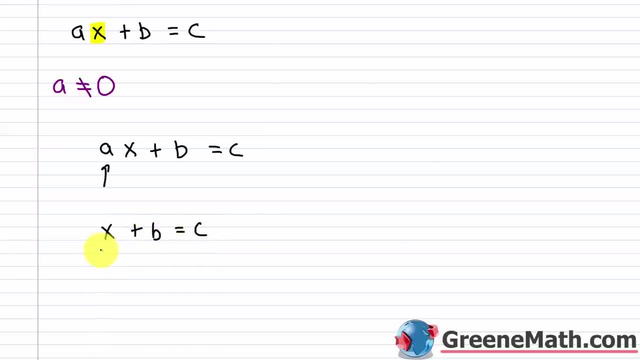 So then plus b equals c. So what I'm saying is you're going to see x plus some number equals c. 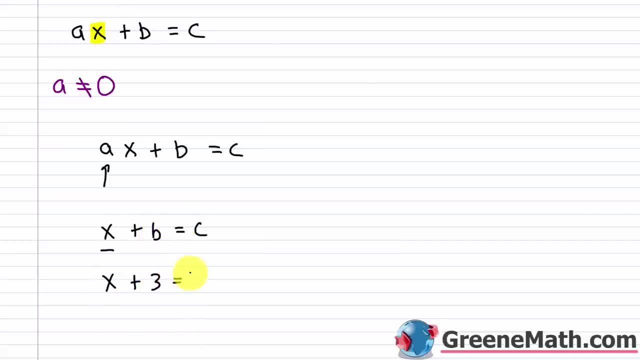 So let's say x plus 3 equals 7, or x minus 4 equals 2. Remember, if I have minus, that's the same thing as plus negative. I could write that as x plus negative 4 equals 2 if I wanted to. 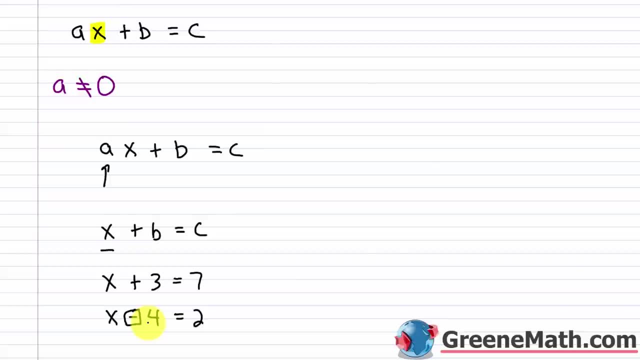 All right, so without further delay, let's talk a little bit about how we solve an equation. So in order to solve an equation of the form that I just showed you, we're going to use three properties. So the first one is very, very simple. It's the fact that a number plus its opposite is always 0. So for example, something like 3 plus negative 3 is 0, right? The opposite of 3 is negative 3. 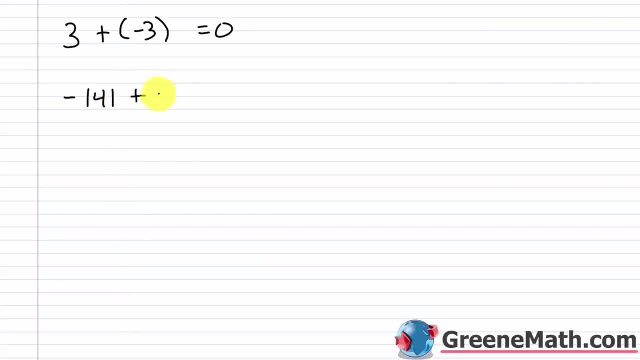 Or negative 141 plus its opposite, which is positive 141, is also 0. 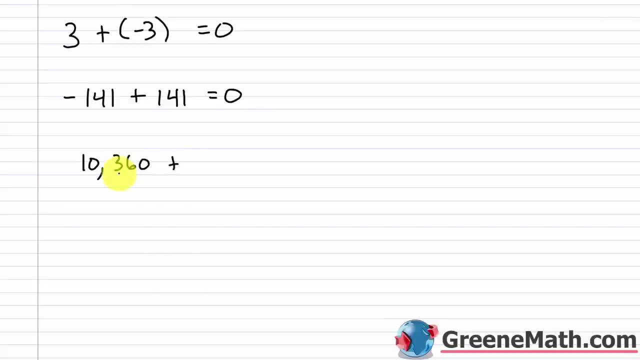 Or 10,360. Plus the opposite of that, which is negative 10,360, is 0. 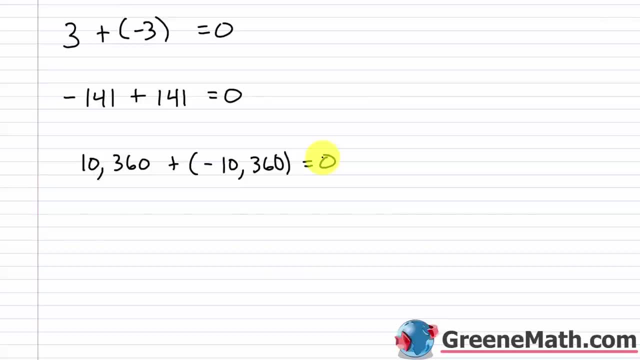 Very, very simple property, but you need to remember that. Now, the other one is that if you add 0 to a number, it remains unchanged. It's called the additive identity, right? So 0, when added to a number, leaves the number unchanged. 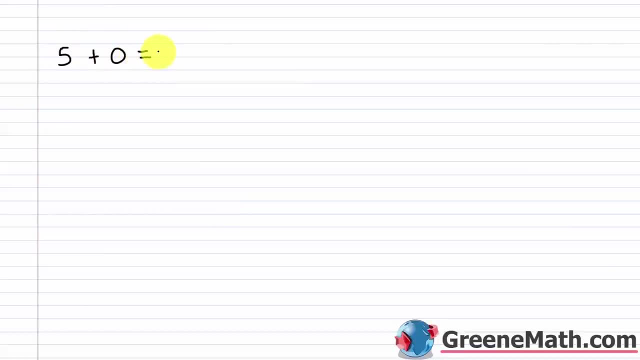 So for example, 5 plus 0 equals 5. 6 plus 0 equals 6. 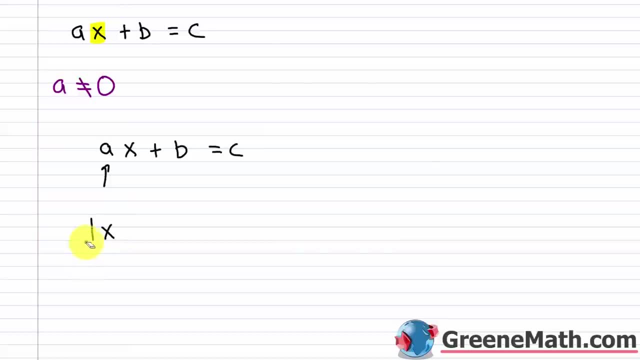 So if you see 1 times x, or 1 is the coefficient of x, you can just write that as x. okay, You don't need to put the 1 next to it, and majority of the time you're not going to. 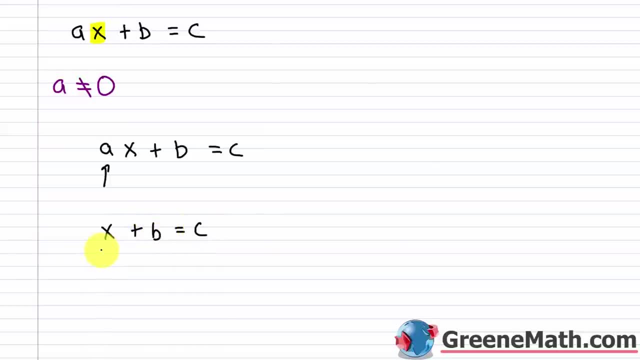 So then plus b equals c. So what I'm saying is you're going to see: x plus some number equals c. So let's say x Plus 3 equals 7, or x minus 4 equals 2.. Remember, if I have minus, that's the same thing as plus negative, right? 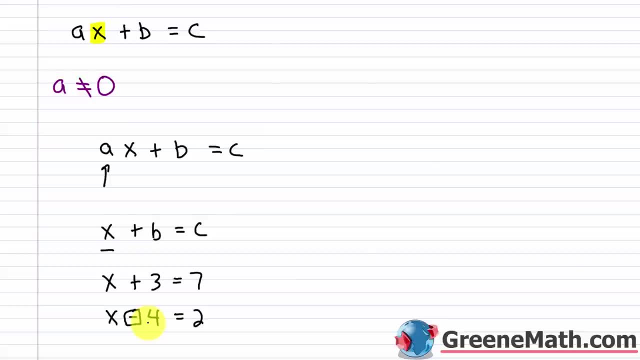 I could write that as x plus negative 4 equals 2, if I wanted to. All right, so without further delay, let's talk a little bit about how we solve an equation. So, in order to solve an equation of the form that I just showed you, we're going to use three properties. 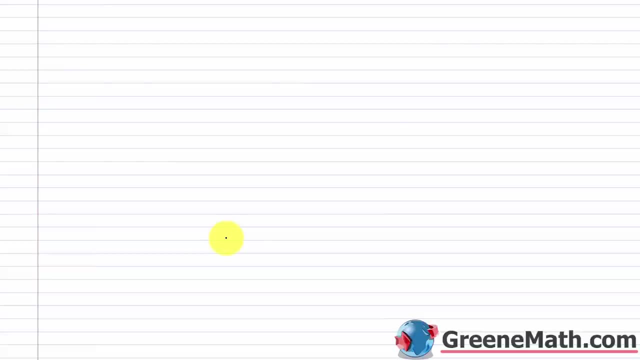 So the first one is very, very simple. It's the fact that a number plus its opposite is always 0. So, for example, something like 3 plus negative 3 is 0, right. The opposite of 3 is negative 3.. 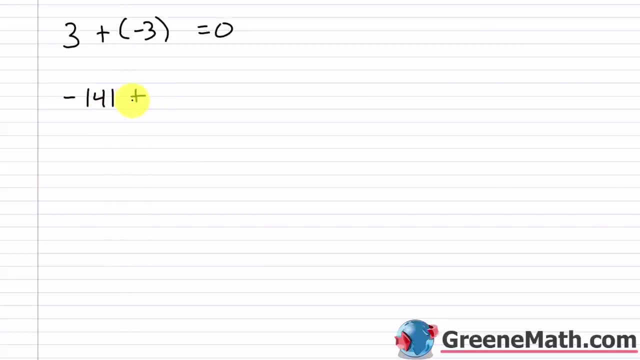 Or negative: 141 plus its opposite, which is positive, 141, is also 0.. Or 10,360 plus the opposite of that which is negative: 10,360, is 0.. Very, very simple property, but you need to remember that. 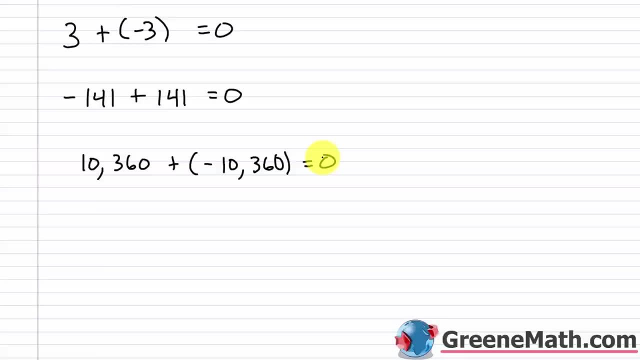 Now the other one is that if you add 0, to a number, it remains unchanged. It's called the additive identity right. So 0,, when added to a number, leaves the number unchanged. So, for example, 5 plus 0 equals 5.. 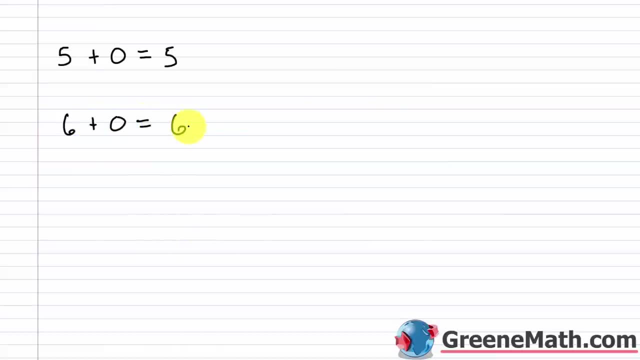 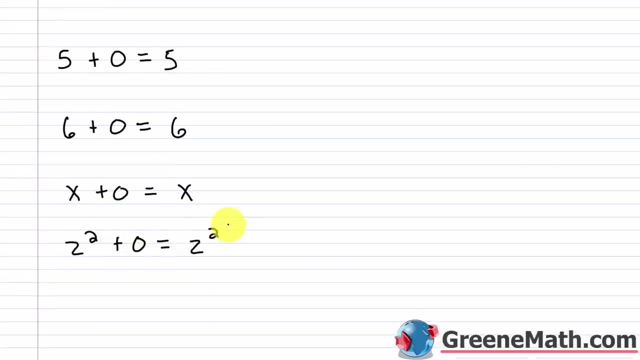 6 plus 0 equals 6.. x plus 0 equals no different, because we have a variable: x z squared plus 0 equals z squared. Okay, So very important that you understand those two properties. Now, the most important property that you're going to learn: 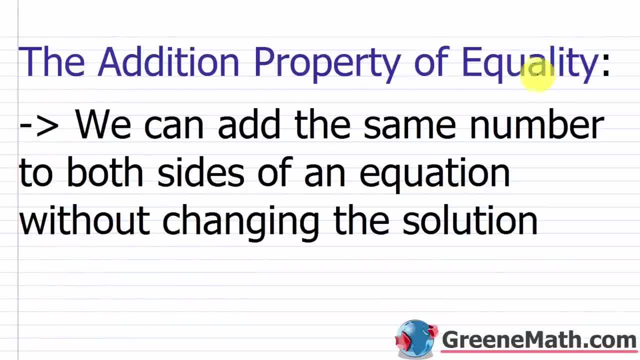 and you definitely want to write this down- is called the addition property of equality, And in fact that's the title of this video. So this tells us that we can add the same number to both sides of an equation without changing the solution. 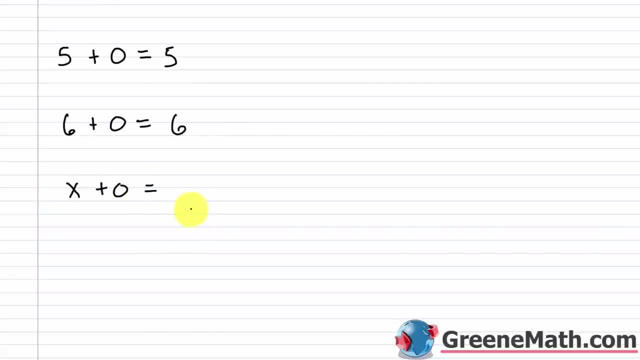 X plus 0 equals, no different because we have a variable, x. Z squared plus 0 equals z squared. 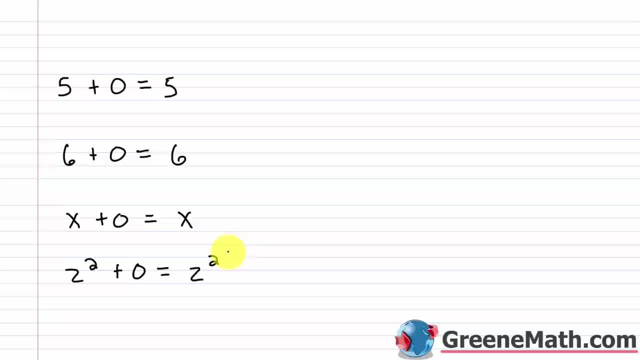 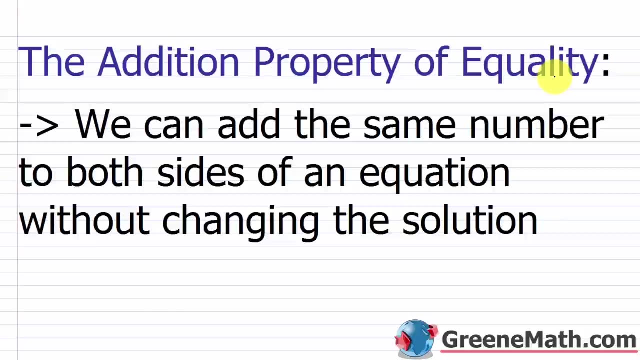 Okay, so very important that you understand those two properties. Now, the most important property that you're going to learn, and you definitely want to write this down, is called the addition property of equality. And in fact, that's the title of this video. 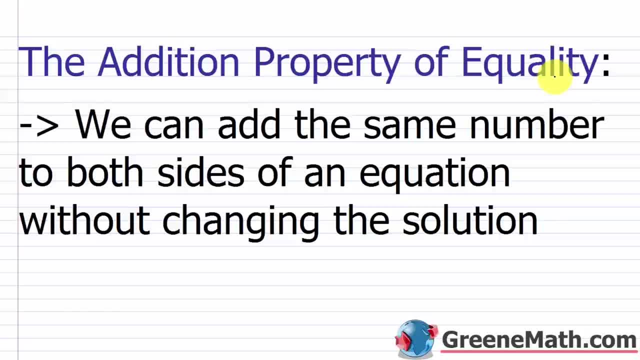 So this tells us that we can add the same number to both sides of an equation without changing the solution. 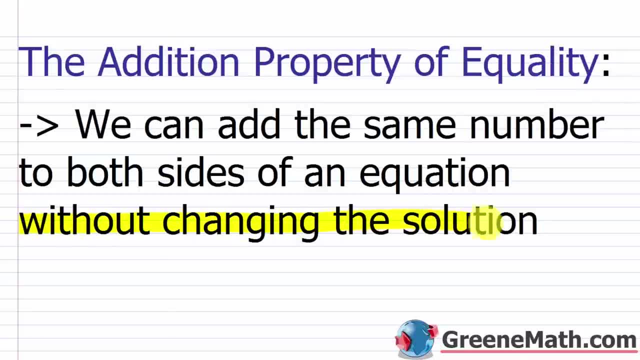 So here's the key, without changing the solution. So I'm going to change what the equation looks like, but the solution, meaning the number that I plug in for the variable that makes it true, is not going to change. 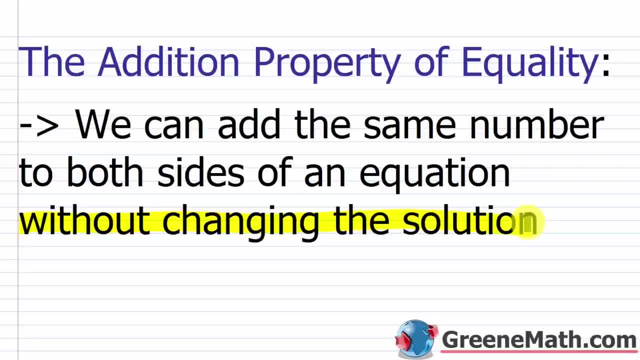 So my original equation that I have has the same solution as the modified one. 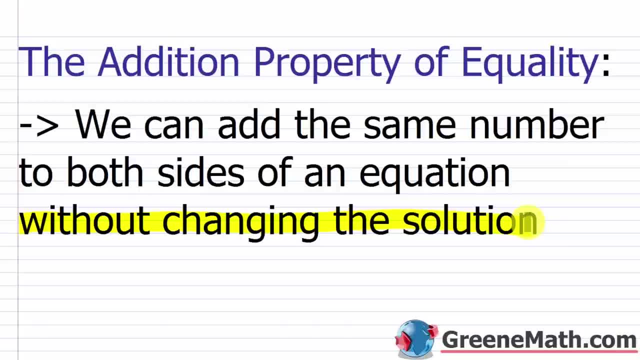 And that's very important because I want to know that the answer that I get in the end works in the original equation. 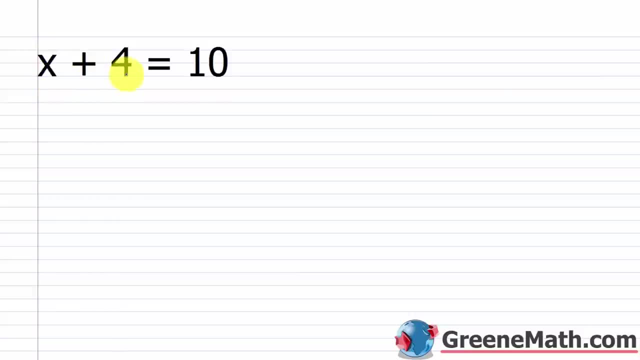 So let's start off with a basic example. We have x plus 4 equals 10. And in the world of solving equations, it doesn't get any easier. So I want to start out with just telling you that your ultimate goal, your number one goal, is to isolate the variable. So I'm always going to start out by just highlighting this or circling it so that I can mentally prepare myself to say, hey, I want to isolate x. 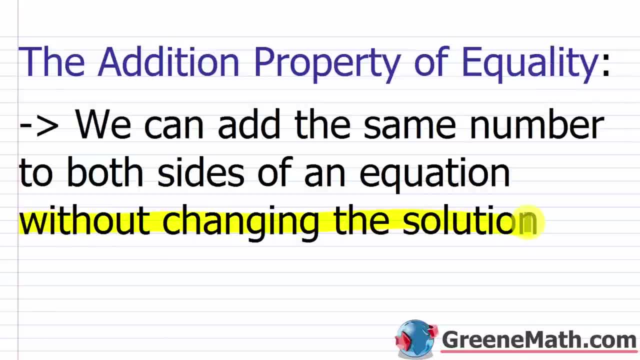 So here's the key, without changing the solution. So I'm going to change what the equation looks like, but the solution, meaning the number that I plug in for the variable that makes it true, is not going to change. So my original equation that I have. 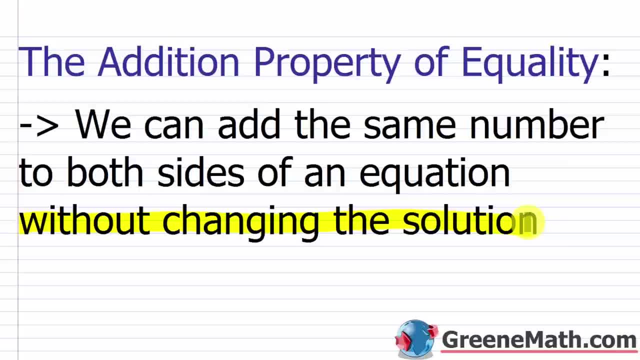 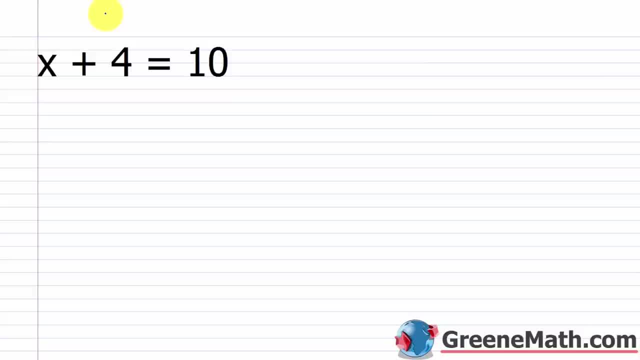 has the same solution as the modified one, And that's very important because I want to know that the answer that I get in the end works in the original equation. So let's start off with a basic example. We have: x plus 4 equals 10.. 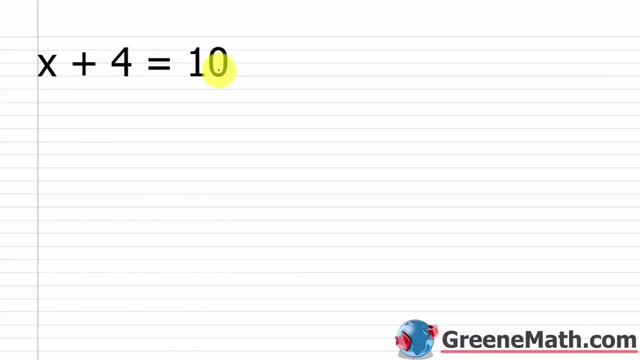 And in the world of solving equations, it doesn't get any easier. So I want to start out with just telling you that your ultimate goal, your number one goal, is to isolate. So I'm always going to start out by just highlighting this. 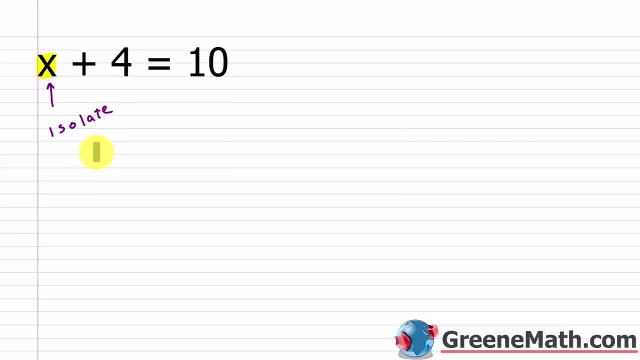 or circling it, so that I can mentally prepare myself to say, hey, I want to isolate x. So what I mean by isolating x? my goal at the end is to have x by itself on one side of the equation. It could be on the left, it could be on the right. 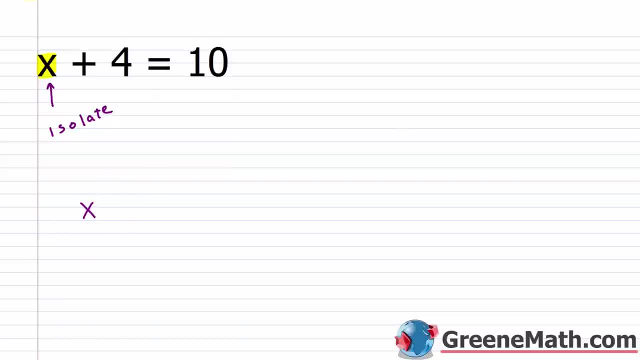 but nothing else can be over there with x. I want x to be equal to some value, to some number. This is going to end up being my solution. x equals some number. that number is the solution, the number that I can plug in for x. 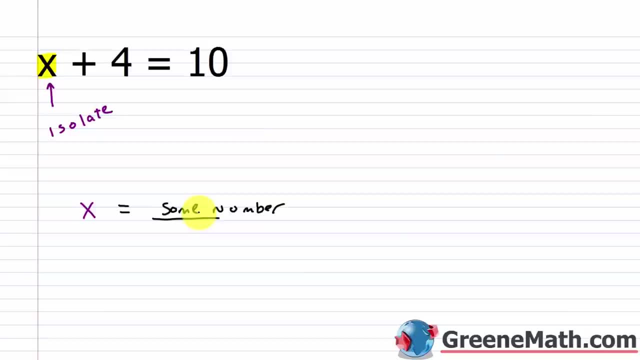 and it should result in a true statement, provided I did my work correctly. So how do we go about isolating x? How do I get x by itself on one side? Well, I want you to look at what's being done to x. 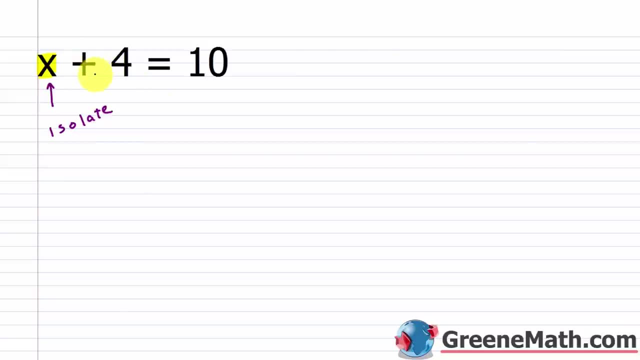 Right now we have 4 that's being added right, So x plus 4.. And think back a moment ago when I told you that if you add 4, if I have 4, plus negative 4, I get 0.. 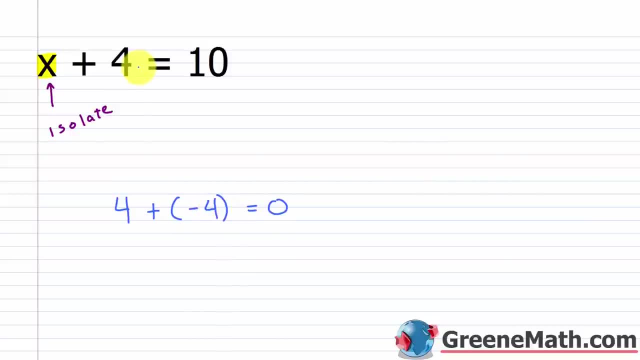 Right, I get 0.. So what happens if I add negative 4 to the left side of the equation? Well, let's do that real quick. So we would have x plus 4 plus negative 4 equals, and then over here we have 10.. 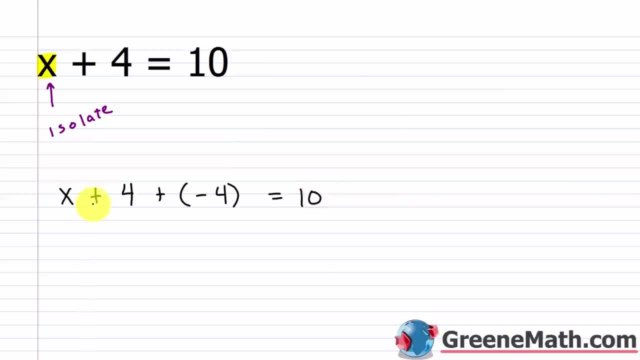 Now, on the left side of the equation, if I simplify 4 plus negative, 4 is 0. So I'm going to rewrite this as: x plus plus 0 equals 10.. Now x plus 0, as I just told you. 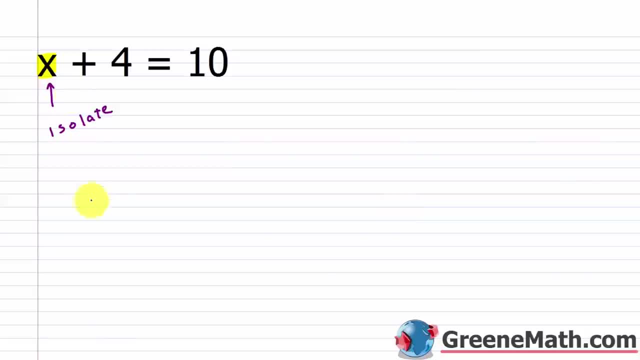 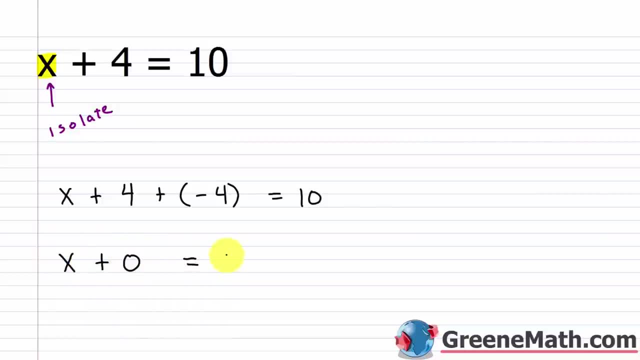 this as X plus 0 equals 10 now X plus 0 as I just told you if you add 0 to a number it remains unchanged same thing with a 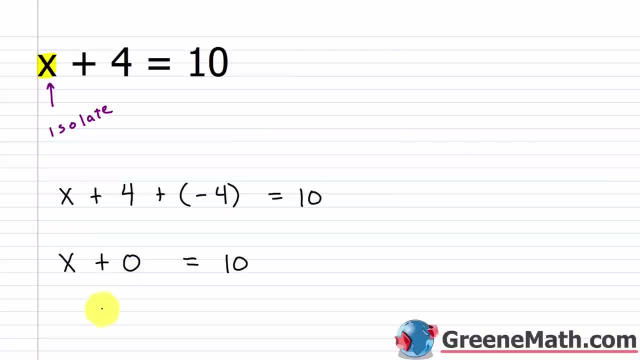 variable so X plus 0 is just X right if I was to simplify so now X is by itself 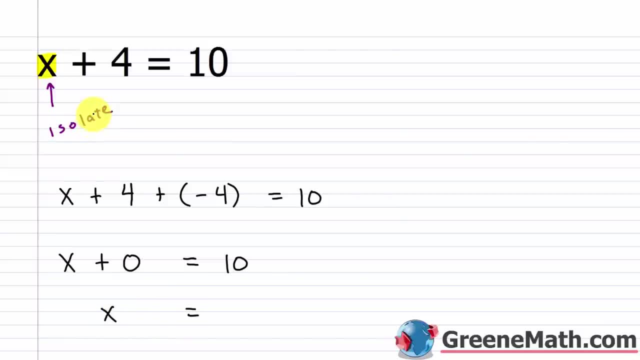 I've met my goal to isolate but there's a problem I can't just go around adding stuff to one side of the equation to make it legal to maintain my solution I've got to do it to both sides otherwise it will not work so I add a negative 4 over here to the left side and I'm gonna do the same thing on the right side so plus negative 4 so now that I've done that I'm gonna maintain my solution meaning the original. 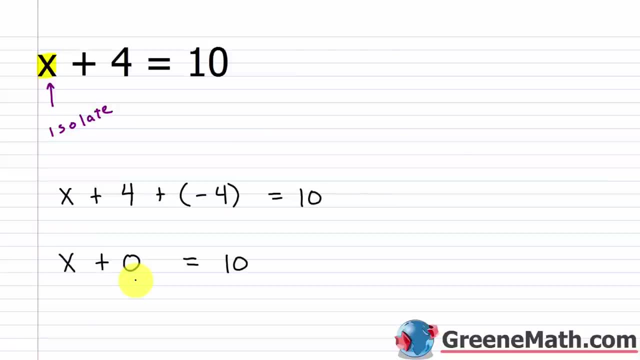 if you add 0 to a number, it remains unchanged. Same thing with a variable. So x plus 0 is just x, right, if I was to simplify. So now x is by itself. I've met my goal to isolate. 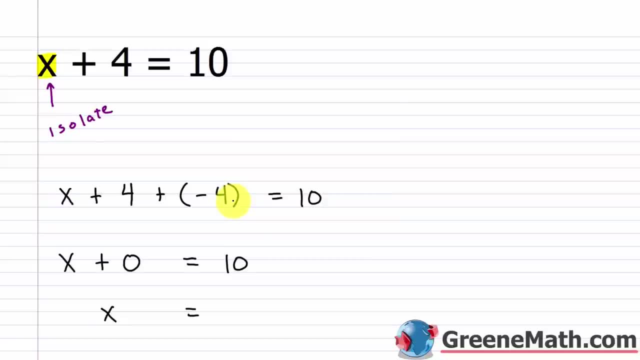 But there's a problem. I can't just go around adding stuff to one side of the equation To make it legal. to maintain my solution, I've got to do it to both sides, Otherwise it will not work. So I add a negative 4 over here to the left side. 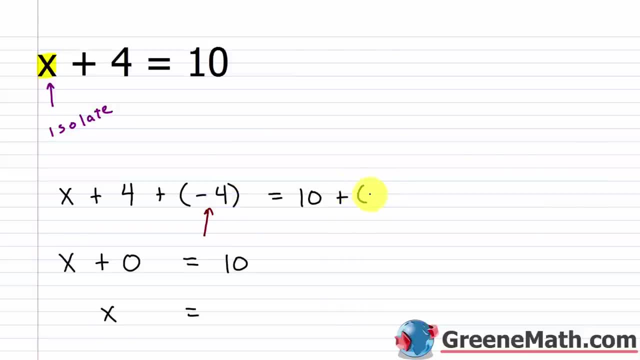 and I'm going to do the same thing on the right side. So plus negative 4.. So now that I've done that, I'm going to maintain my solution, meaning the original solution for x plus 4 equals 10, which you can probably guess is 6 at this point. 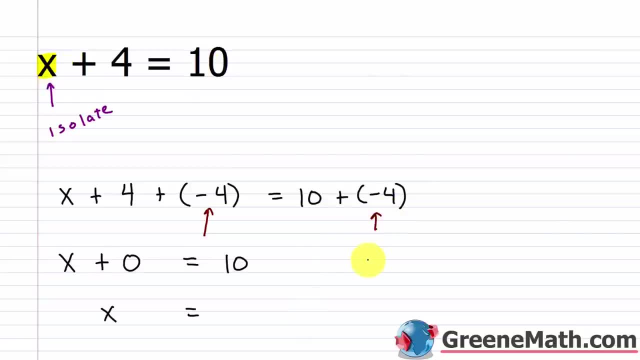 will still be true when I get down here. Throughout the steps. your equation is going to look different each time, but it's going to maintain that same solution, which is what we need. So if I add negative 4 and 10, in this step here, 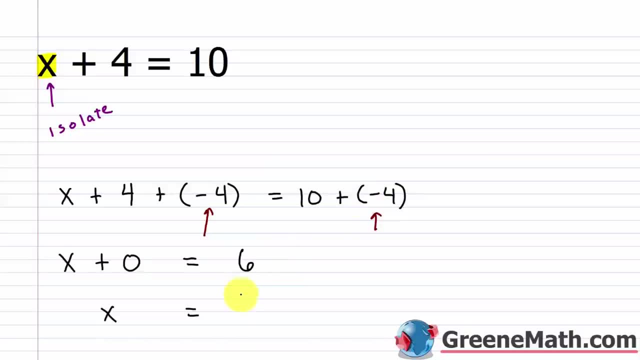 instead of writing 10,, I'm going to have 6.. And then down here I would write 6 again, because x plus 0 equals 6, then we have x equals 6.. So once I get to this point where x equals some number, 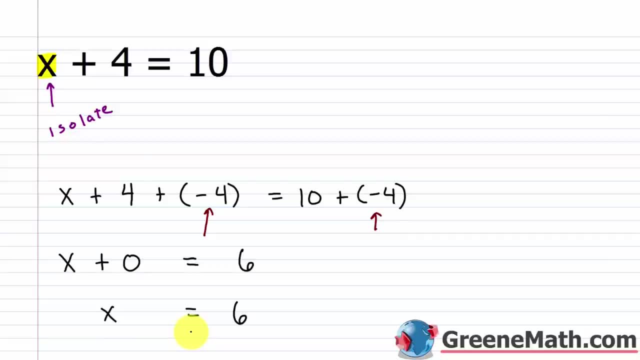 I have my solution, I have my value, that when it replaces the variable, it gives me a true statement. So x equals 6.. So we already know how to check and see if we got the right answer. I take a 6.. 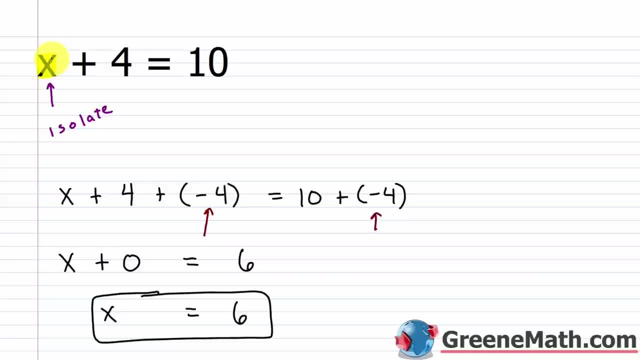 I plug it back in for x And I see if I get the same value on the left and the right side. So let me erase this And I would just plug in a 6 for x, So I would have 6 plus 4 equals 10.. 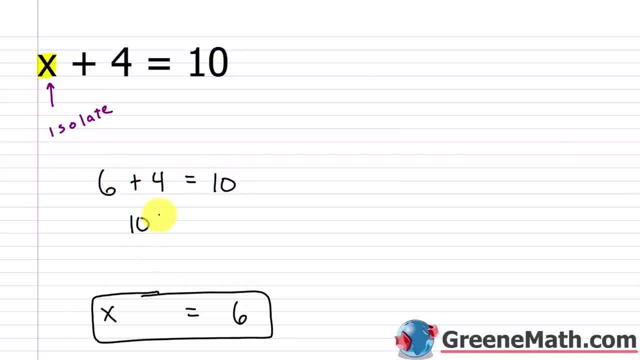 We all know that 6 plus 4 is 10.. So the value on the left is 10.. The value on the right is 10.. And so we get a true statement, right? So x equals 6 is the correct solution here, right? 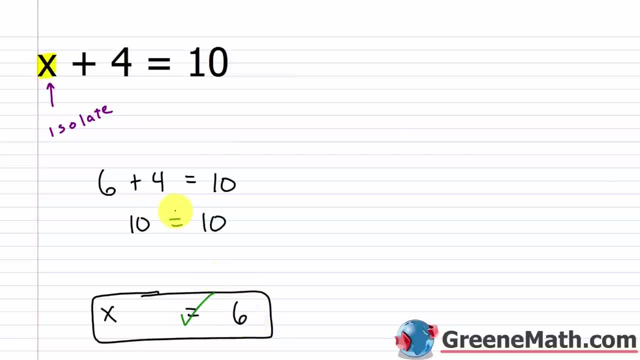 Because, again, when I plug a 6 in for x, I end up with the same value on the left as on the right. Now let's say, for example, you didn't get the right answer. Let's say, you goofed up. 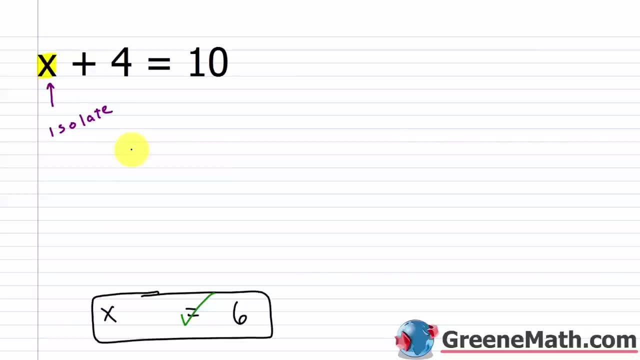 And you understood the principle here, but you missed a step. Let's say you did x plus 4. And you subtracted 4 away, or you added negative 4.. Again, those are the same thing. So sometimes you'll see me put minus 4.. 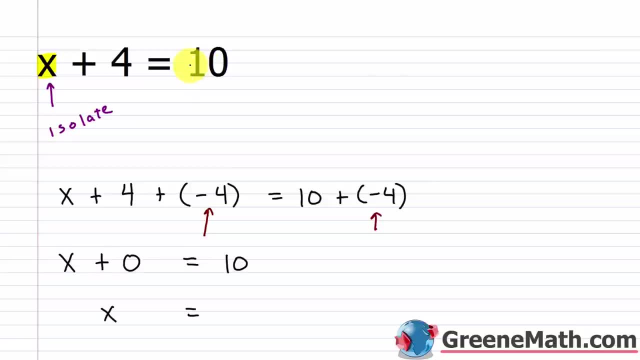 solution for x plus 4 equals 10, which you can probably guess is 6 at this point, will still be true when I get down here. Throughout the steps your equation is going to look different each time but it's going to maintain that same solution which is what we need. So if I add negative 4 and 10 in this step here instead of writing 10 I'm going to have 6 and then down here I would write 6 again because x plus 0 equals 6 then we have x equals 6. So once I get to this point where x equals some number I have my solution, I have my value that when it replaces the variable it gives me a true statement. So x equals 6. So we already know how to check and see if we got the right answer. I take a 6, I plug it back in for x and I see if I get the same value on the left and the right side. Let me erase this and I would just plug in a 6 for x. So I would have 6 plus 4 equals 10, we all know that 6 plus 4 is 10, so the value on the left is ten, the value on the right is ten, the value on the left is ten, the value on the left is ten, on the right is 10 and so we get a true state right so X equals 6 is the correct solution here right because again when I plug a 6 in for X I end up with the same 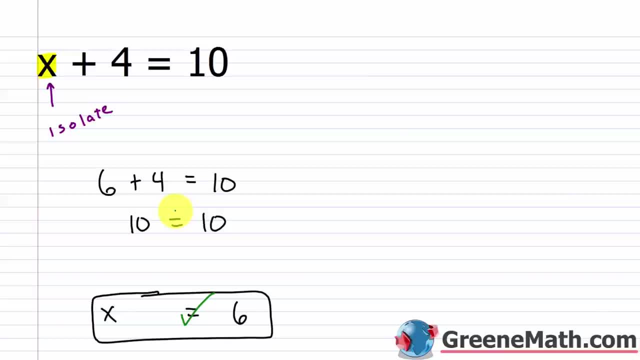 value on the left as on the right now let's say for example you didn't get the right answer let's say you goofed up and you understood the principle here but you missed a step let's say you did X plus 4 and you subtracted 4 away or you added negative 4 again those are the same thing so sometimes you'll see me put minus 4 sometimes you'll see me put plus negative 4 same exact thing then equals let's say you just put 10 and I forget to add negative 4 on this side so this cancels and I have X and now I'm saying X equals 10 well X doesn't equal 10 but when you go back and check it you're gonna figure out hey I made a mistake 10 plus 4 is 14 14 is not equal to 10 so that's how you catch your simple mistakes especially when you're trying to figure out how to solve a problem and how to 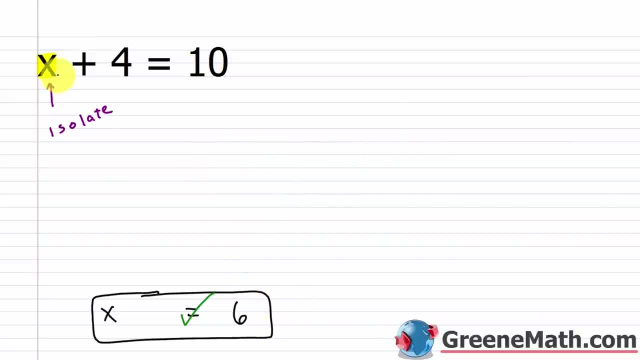 solve it in the beginning you take your value plug it back in for the variable and see if the left and the right side are equal very important you check your work at this stage of the game all right let's take a look at another one all right let's say we have X minus 7 equals negative 12 so again our goal is to 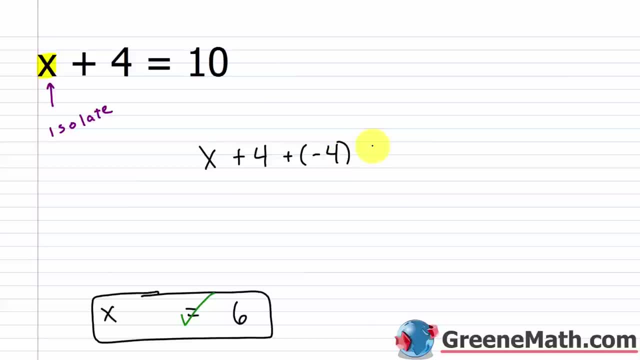 Sometimes you'll see me put plus negative 4.. Same exact thing, Then equals. let's say you just put 10. And I forget to add negative 4 on this side. So this cancels and I have x, And now I'm saying x equals 10.. 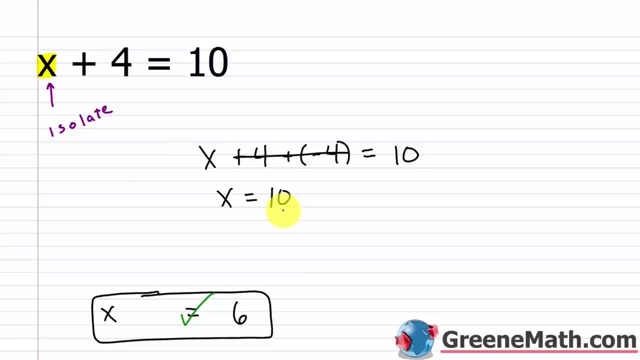 Well, x doesn't equal 10.. But when you go back and check it you're going to figure out. hey, I made a mistake. 10 plus 4 is 14.. 14 is not equal to 10.. So that's how you catch your simple mistakes. 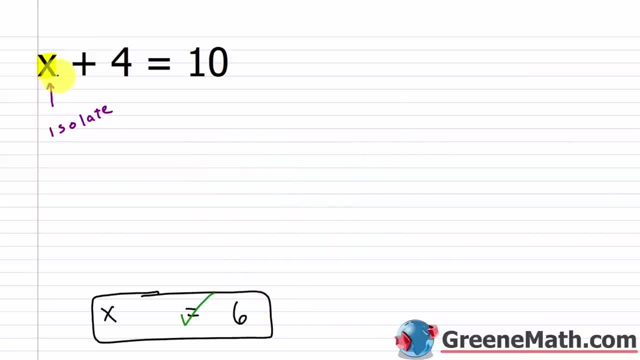 especially in the beginning. You take your value, plug it back in for the variable and see if the left and the right side are equal- Very important, you check your work at this stage of the game. All right, let's take a look at another one. 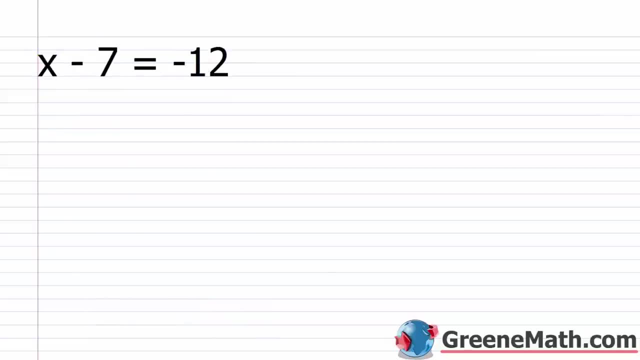 All right, let's say we have x minus 7 equals negative 12. So, again, our goal is to isolate the variable. We want to isolate x, And let me highlight it. So what's being done to x right now? 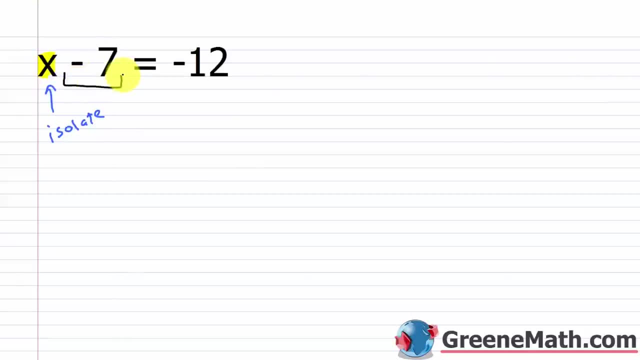 I always think about: okay, what's being done? Well, I'm subtracting 7 away. I want x by itself. So remember, I can use that trick where I have x plus 0.. Well, if I have x minus 7,? 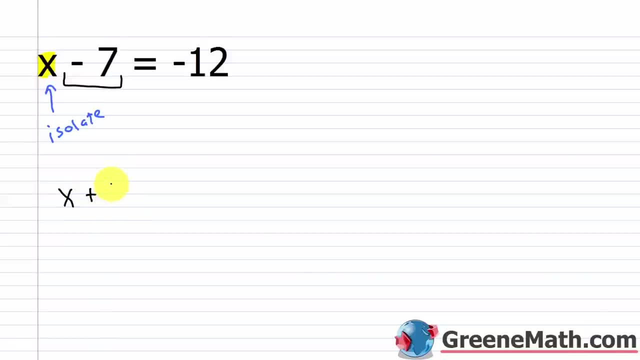 and it might make you more comfortable to write that as x plus negative 7,. what can I add over here? I can add x plus 0 over here to get x plus 0, right, Because we know that simplifies to x. 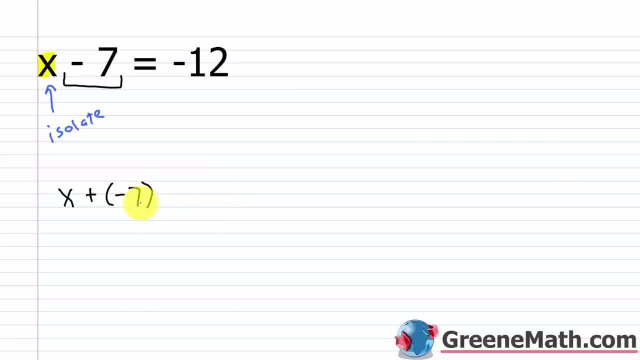 and I'd have x isolated on one side. Remember if I had the opposite of negative 7, which is positive 7, negative 7 and positive 7 would give me 0. So plus 7. Okay, then equals negative 12.. 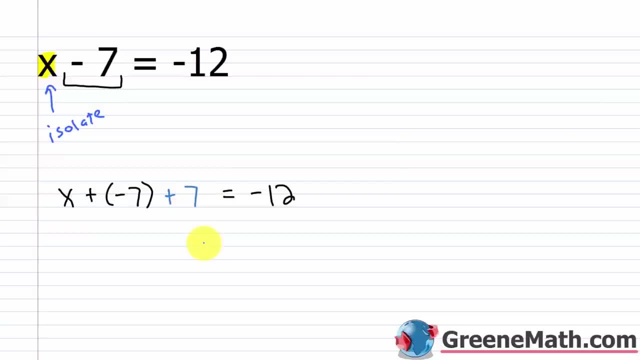 But remember, I can't just go around adding whatever I want to one side of the equation. If I'm going to do that, I've got to do it to the other side so that I maintain my solution. So plus 7 over here as well. 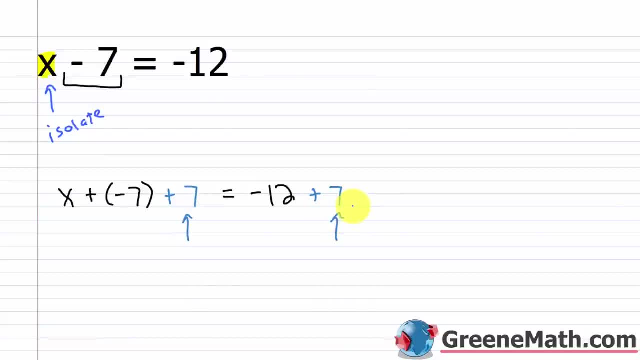 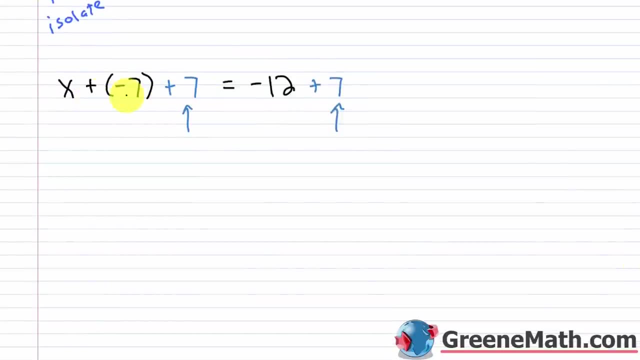 So now we've got it on this side and this side, so we are good to go. All right, let's scroll down a little bit and we'll have x plus negative 7 plus 7.. So we know that negative 7 plus 7 is 0,. 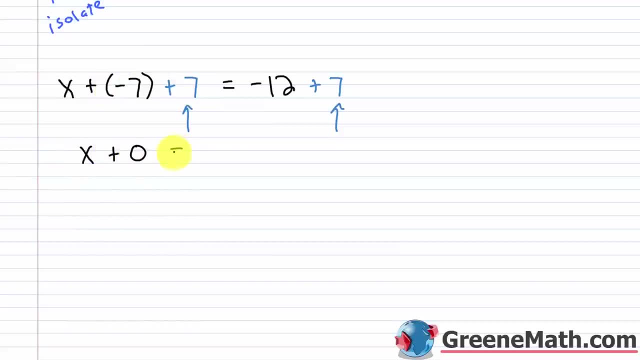 so this would be x plus 0.. And this equals negative 12 plus 7, which is negative 5.. I can simplify x plus 0 to just x, and this equals negative 5.. And in the future equations I'm going to stop writing x plus 0. 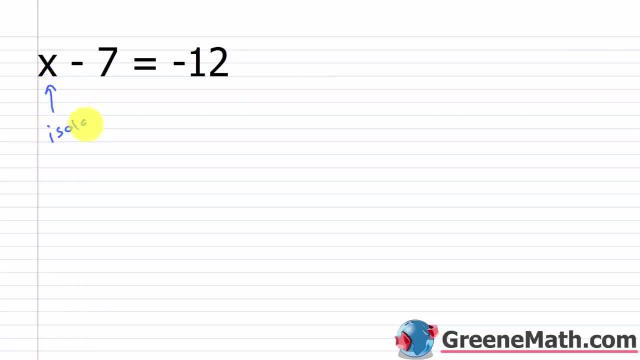 isolate the variable we want to isolate X and let me highlight it so what's 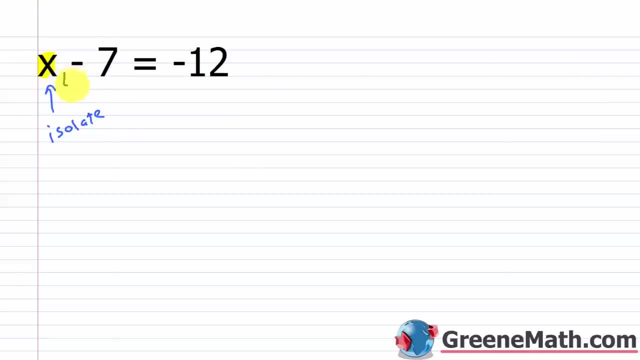 being done to X right now I always think about okay what's being done right now but what's being done is I'm subtracting 7 away I want X by itself so remember I can use that trick where I have X plus 0 well if I have X minus 7 and it might make you more comfortable to write that as X plus negative 7 what can I add over here to get X plus 0 right because we know that simplifies to X and I'd have X isolated on one side remember if I had the opposite of negative 7 which is positive 7 negative 7 and positive 7 would give me 37 and then the final sumx is showing me the total addition今 opposite of negative 7 which is positive 7 negative 7 and positive 7 would give me 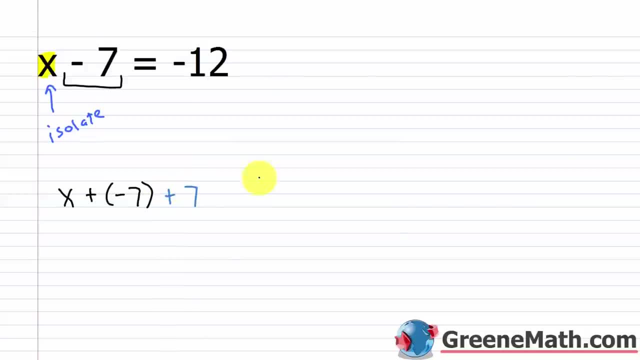 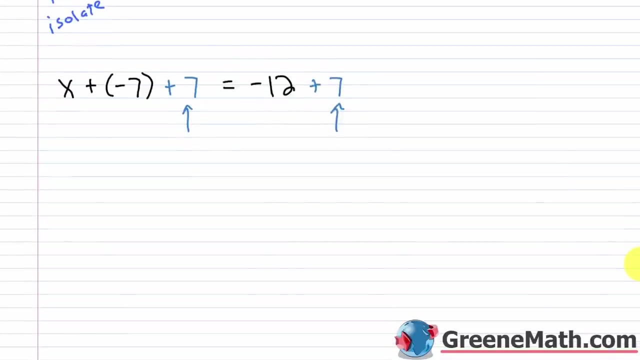 zero. So plus seven, okay, then equals negative 12. But remember, I can't just go around adding whatever I want to one side of the equation. If I'm going to do that, I've got to do it to the other side so that I maintain my solution. So plus seven over here as well. So now we've got it on this side and this side. So we are good to go. All right, let's scroll down a little bit and we'll have x plus negative seven plus seven. So we know that negative seven plus seven is zero. 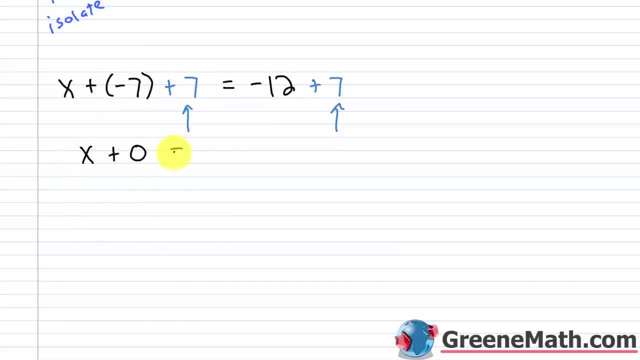 So this would be x plus zero. And this equals negative 12 plus seven, which is negative five. I can simplify x plus zero to just x. And this equals negative five. And in the future equations, I'm going to stop writing x plus zero, we know that x plus zero is just x. So I'm just going to line out this and then we're going to just say, okay, that's x now. 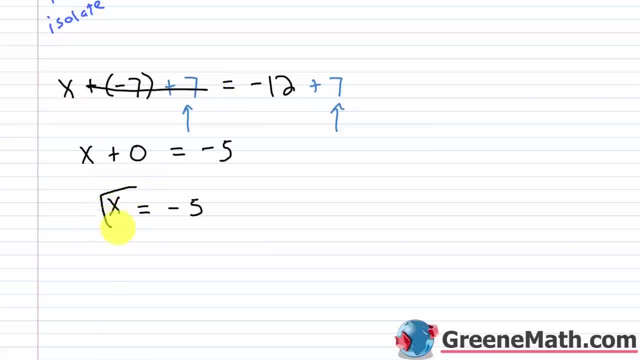 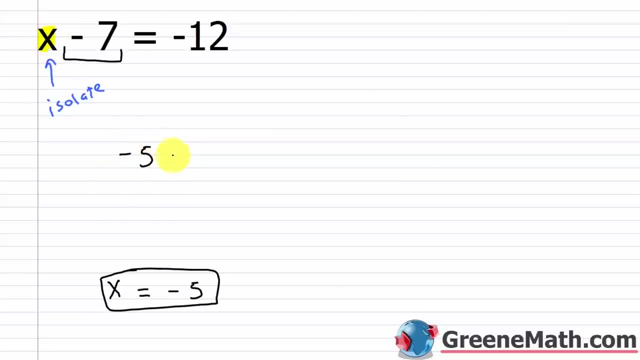 All right, so we get our solution, which is x equals negative five. And we can check it by plugging in a negative five for x. So if I plug a negative five in there, I'd have negative five minus seven equals negative 12. Negative five minus seven is negative 12. You get negative 12 equals negative 12. And so yes, my solution here of x equals negative five 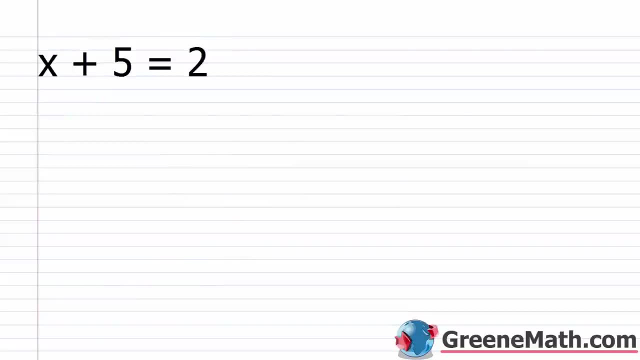 is correct. All right, what about x plus five equals two? Well, again, I want to isolate my variable x. So I want to isolate my variable x, which is negative five. And so I'm going to 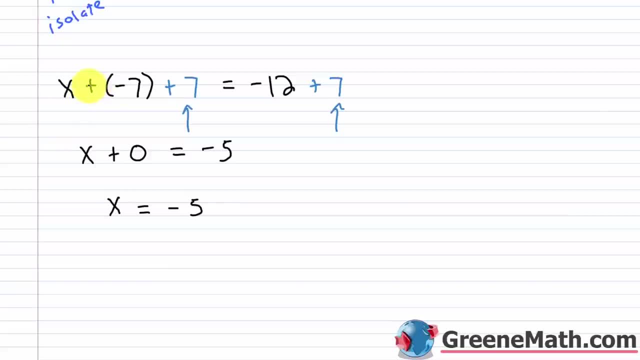 We know that x plus 0 is just x, so I'm just going to line out this and then we're going to just say, okay, that's x now. All right, so we get our solution, which is: x equals negative 5.. 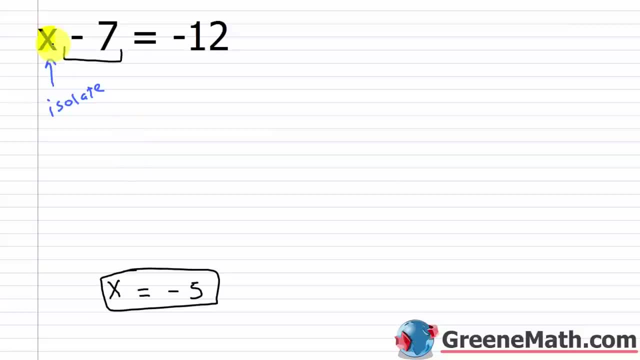 And we can check it by plugging in a negative 5 for x. So if I plug a negative 5 in there, I'd have negative. 5 minus 7 equals negative 12.. Negative 5 minus 7 is negative 12.. 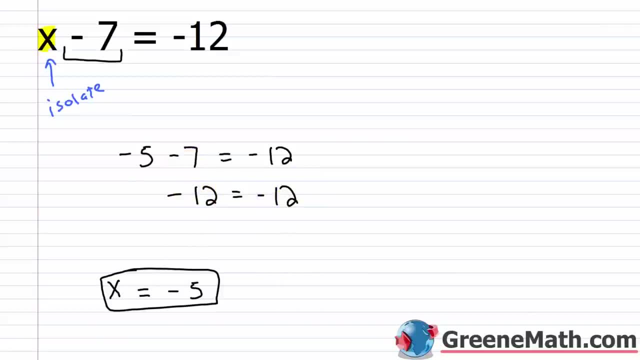 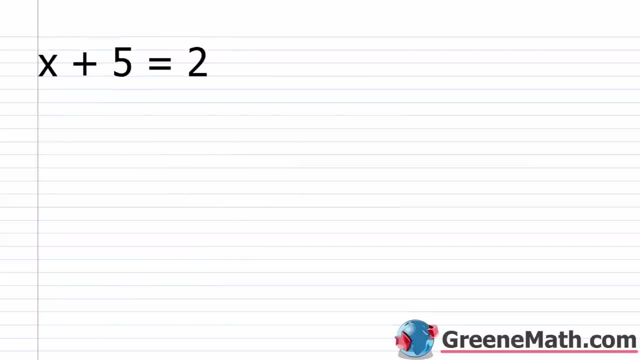 You get: negative 12 equals negative 12.. And so, yes, my solution here of x equals negative 5 is correct. All right, what about x plus 5 equals 2?? Well, again, I want to isolate my variable x. 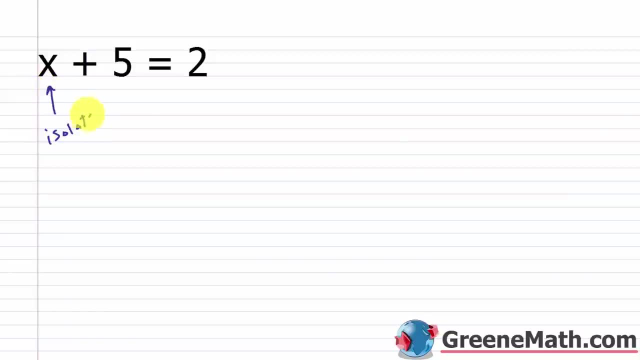 So I want to isolate, isolate, And so let me highlight this guy right here. And in order to do that again, if I'm adding 5 to x, what can I do to make that 5 go away? Well, if I have 5 and I add negative 5,. 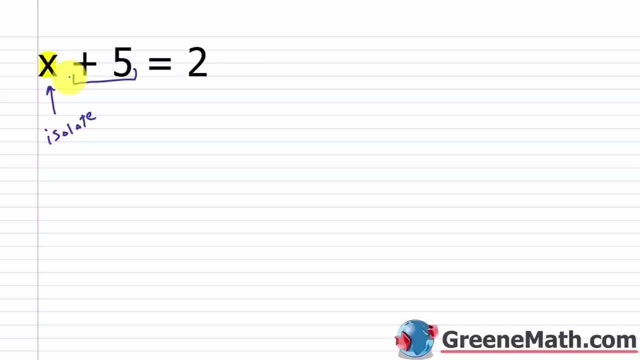 or I subtract away 5, again, that's the same thing. that's going to go away. right, That 5 will disappear. Here I'll just have x. So if I have x plus 5 plus negative 5,, 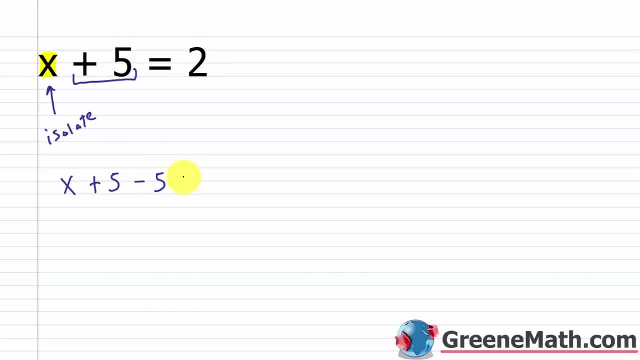 or I can write minus 5, but again, if I'm doing that over here, if I'm subtracting 5 away, I've got to do the same thing over here. I've got a minus 5 over here as well. 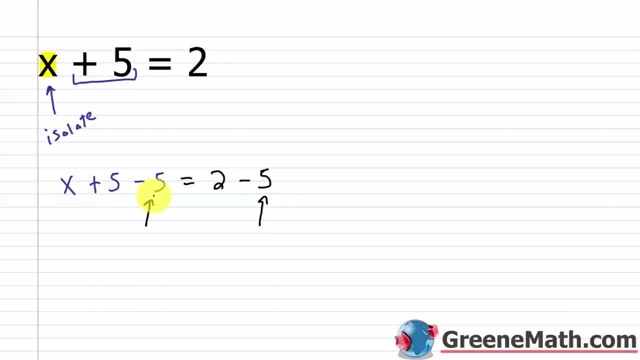 So now I can go through and simplify. So 5 minus 5 is 0. So I'm not going to write x plus 0. You know, that's just going to simplify to x. So I'm just going to cross this out and just put that this is x. 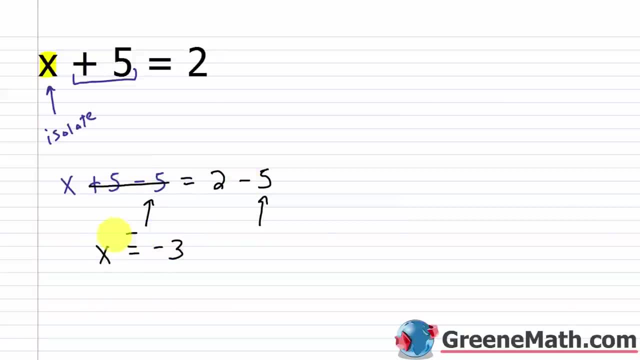 And this equals 2 minus 5.. 2 minus 5 is negative 3. So we get x equals negative 3.. Again, you can plug negative 3 back in for x and show that we get a true statement. So you'd have negative 3 there plus 5 equals 2.. 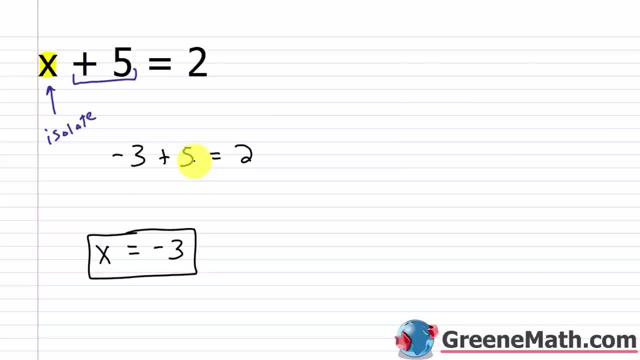 So negative 3 plus 5 is the same thing as 5 minus 3, and we know that's 2.. So we get 2 equals 2. And so again we can say our solution here x equals negative 3, is correct. 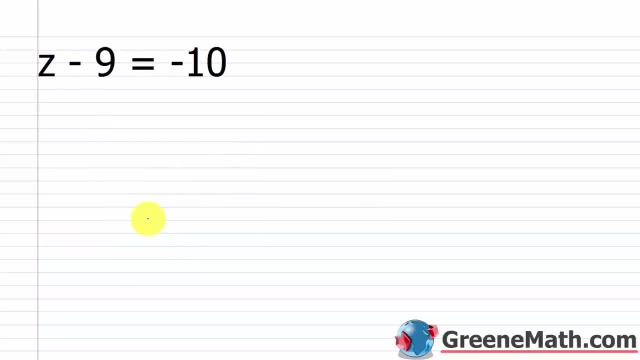 All right, let's take a look at the final problem here. So we have z minus 9 equals negative 10.. So now my variable is z and I always want to isolate it, And I know a lot of students get confused when they see something other than x at first. 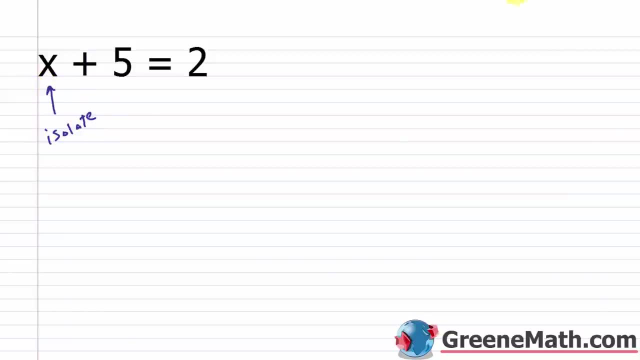 Isolate. Isolate. And so let me highlight this guy right here. And in order to do that, again, if I'm adding five to x, what can I do to make that five go away? Well, if I have five and I add negative five, or I subtract away five, again, that's the same thing, that's going to go away, right? That five will disappear. I'll just have x. So if I have x plus five, plus negative five, or I can write minus five. But again, if I'm doing that over here, if I'm subtracting five away, 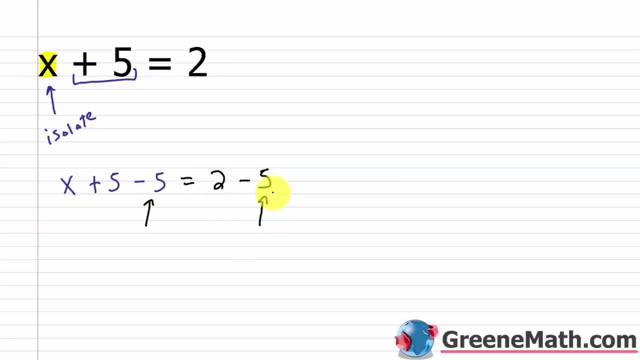 I've got to do the same thing over here. I've got a minus five over here as well. So now I can go through and simplify. So five minus five is zero. So I'm not going to write x plus zero. You know that's just going to simplify to x. So I'm just going to cross this out and just put that this is x. And this equals two minus five is negative three. So we get x equals negative three. Again, you can 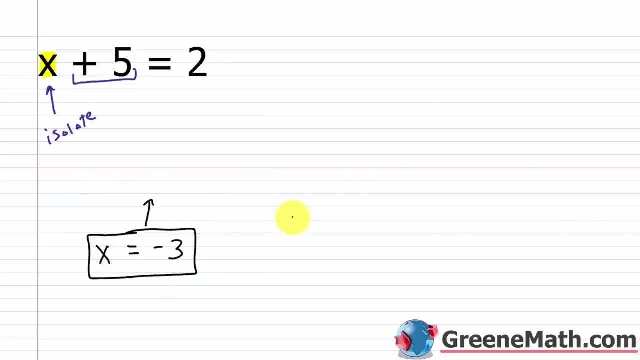 plug negative 3 back in for x and show that we get a true statement so you'd have negative 3 there plus 5 equals 2 so negative 3 plus 5 is the same thing as 5 minus 3 and we know that's 2 so we get 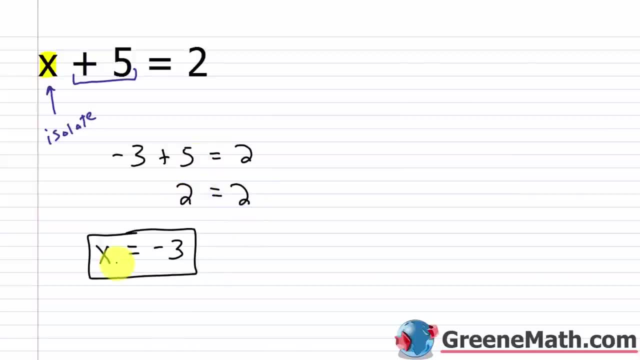 2 equals 2 and so again we can say our solution here x equals negative 3 is correct all right 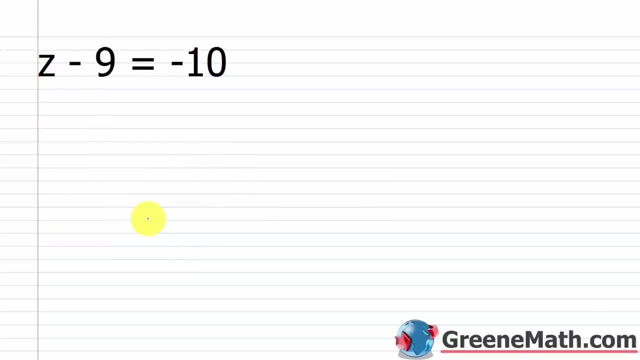 let's take a look at the final problem here so we have z minus 9 equals negative 10 so now my variable is z and i always want to isolate it and i know a lot of students get confused when they see something other than x at first but again your variable can be whatever in this case it's z that's our unknown now to isolate z we look at what's being done to z so right now i'm subtracting 9 away and you can think about that as adding negative 9 if that's more comfortable for you so we'll have z let's go ahead and put plus negative 9 and if i think about this side only 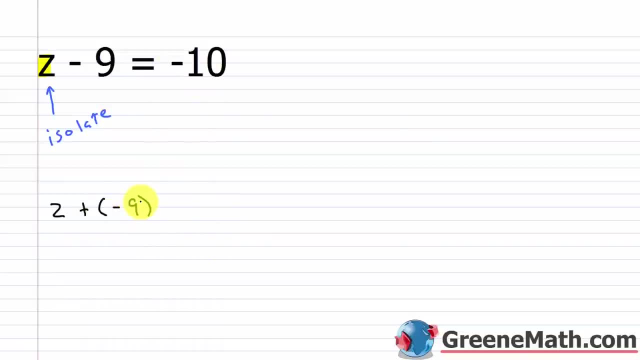 you can think about this side only you can think about this side only forget about this for a second how can i make this negative 9 go away well again if i have negative 9 and i add the opposite of that which is positive 9 negative 9 plus 9 would be 0 so over here this would go away and i would just have z 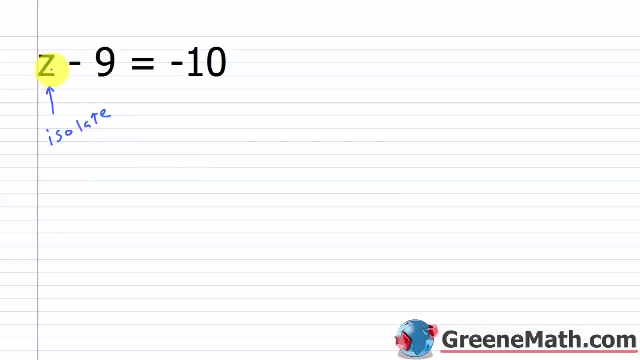 but again, your variable can be whatever. In this case it's z. That's our unknown. Now to isolate z, we look at what's being done to z. So right now I'm subtracting 9 away And you can think about that as adding negative 9. 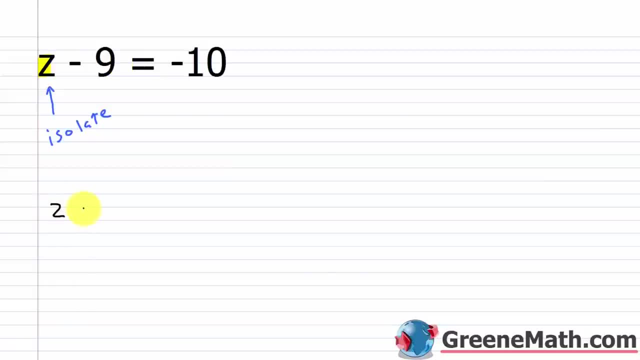 if that's more comfortable for you. So we'll have z. Let's go ahead and put plus negative 9.. And if I think about this side, only forget about this for a second. how can I make this negative 9 go away? 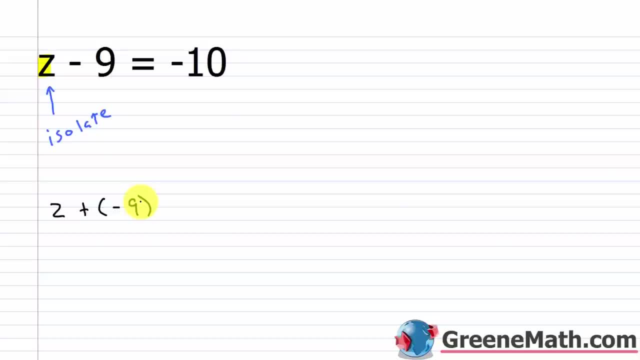 Well, again, if I have negative 9 and I add the opposite of that which is positive 9, negative 9 plus 9 would be 0. So over here this would go away and I would just have z. 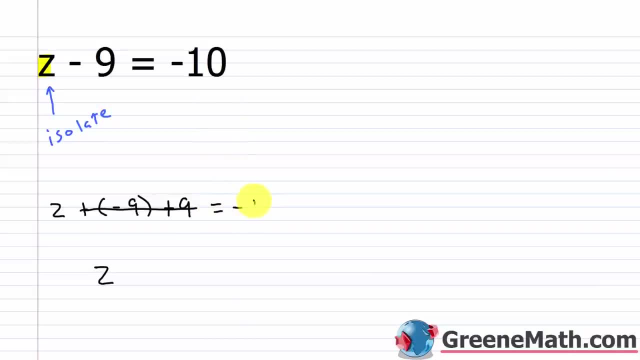 But to make it legal, I've got to also do that same action, which is to add 9 to the right side. So in other words, I added it over here, I've got to add it over here, Otherwise I'm going to end up messing up my solution. 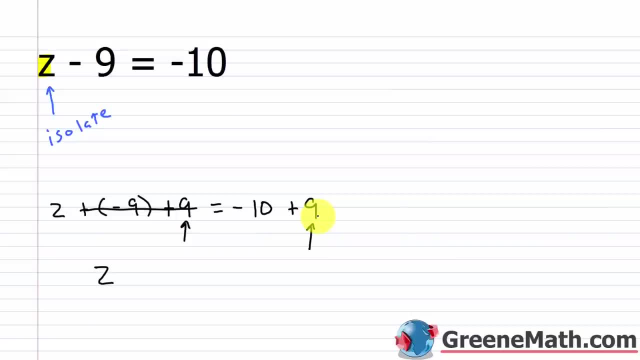 We need our solution to stay the same so we get the right answer. So over here now I would have: z is equal to negative. 10 plus 9 is negative 1.. So that's my solution: z equals negative 1.. Now again, we plug back in for z in the original equation. 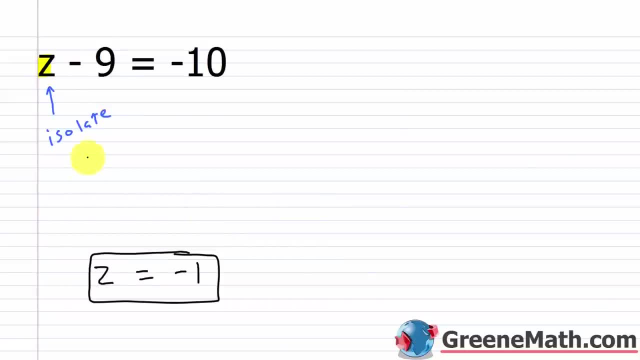 Let me erase this and we'll say, instead of z I'll have: negative 1 minus 9 equals negative 10, and negative 1 minus 9 is negative 10.. Negative 10 is equal to negative 10.. Same value on each side of the equation. 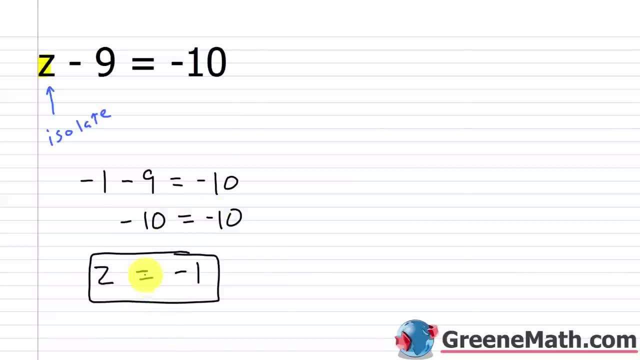 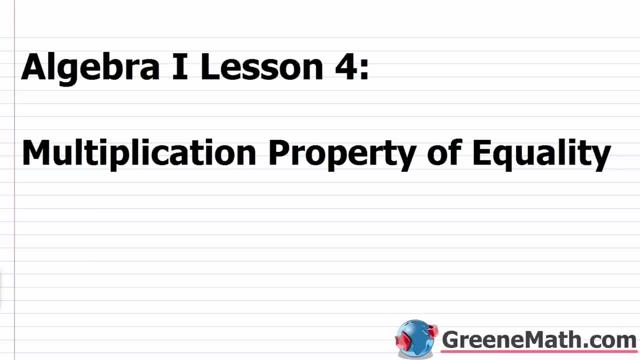 and so we can say that our solution z equals negative 1, is correct. Hello and welcome to Algebra 1,, Lesson 4.. In this video we're going to learn about the multiplication property of equality. So in the last lesson we finally started talking about. 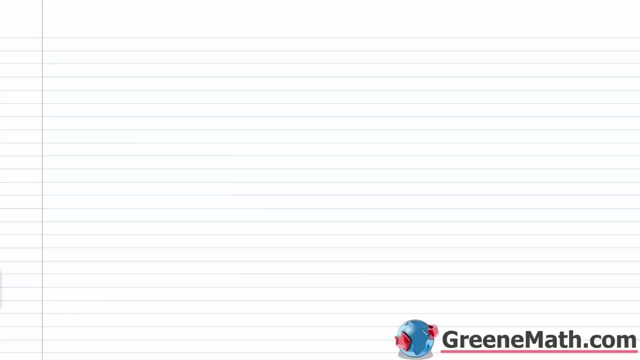 how to solve an equation And we started talking about the first type of equations that we look at, and those are linear equations in one variable. so let me kind of redefine that for you. So a linear equation in one variable looks like this: 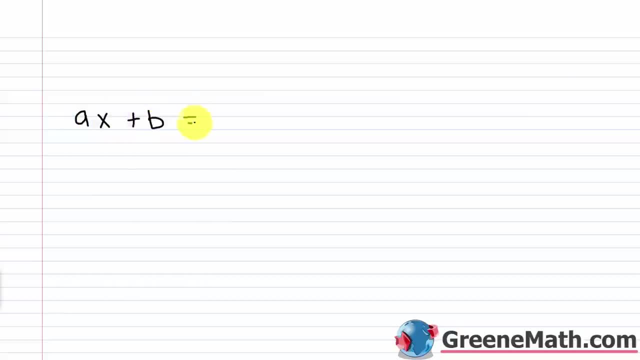 So it's ax plus b equals c, And again your variable doesn't have to be x, but again that's the most commonly used in algebra. so we kind of show that when we show a generic formula Now. I also told you that a, b and c could be any real number. 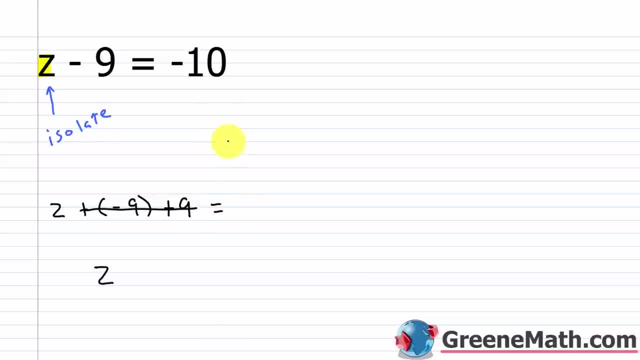 but to make it legal i've got to also do that same action which is to add 9 to the right side so in other words i added it over here i've got to add it over here otherwise i'm going to end up messing up my solution we need our solution to stay the same so we get the right 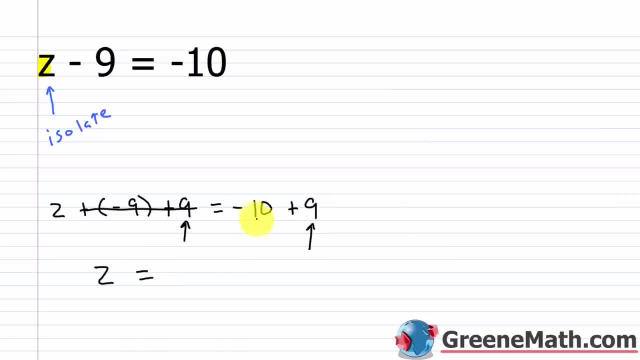 answer so over here now i would have z is equal to negative 10 plus 9 is negative 1 so that's my solution z equals negative 1 now again we plug back in for z in the original equation let me erase this and we'll say instead of z i'll have negative 1 minus 9 equals negative 10 and negative 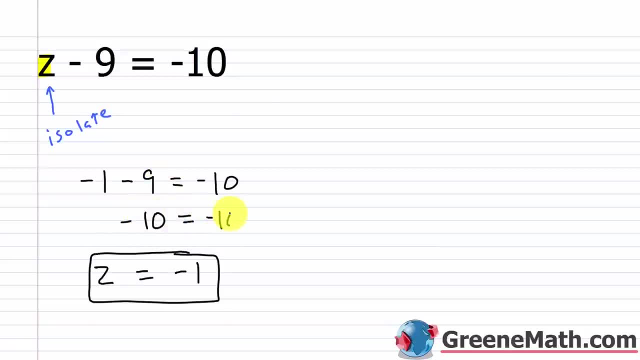 1 minus 9 is negative 10 negative 10 is equal to negative 10 and negative 10 is equal to negative 10 negative 10 same value on each side of the equation and so we can say that our solution 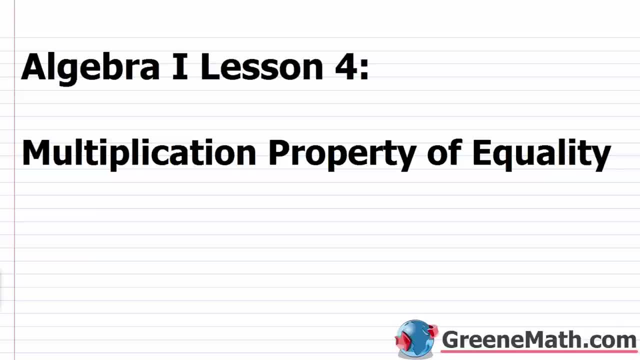 z equals negative 1 is correct hello and welcome to algebra 1 lesson 4 in this video we're going to learn about the multiplication property of equality so in the last lesson we finally started 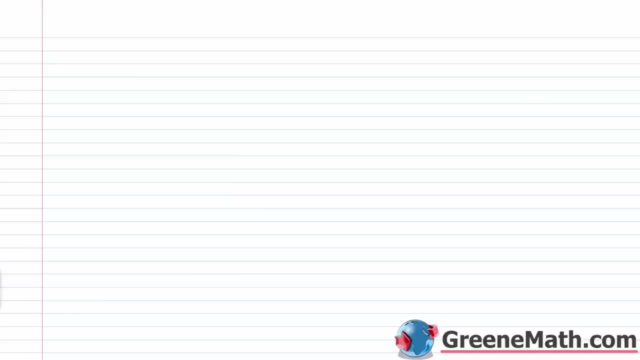 talking about how to solve an equation and we started talking about the first type of equations that we look at and those are linear equations in one variable so let me kind of redefine that for you so a linear equation one variable looks like this so it's ax plus b equals c and again your variable doesn't have to be x but again that's the most commonly used in algebra so we kind of show that when we show a generic formula now i also told you that a b and c could be any real number that you could think of i had one exception to that your value for a which is the coefficient of x cannot be zero so a cannot be zero because again if zero multiplies x x is going to disappear right zero times anything is always zero so we can't have x dropping out because this is an equation and we need to have a variable so other than that again a b and c can be anything that you want it to be now specifically in the last lesson we looked at the case where a was one right we had one x plus b equals c one times x anything times one is just itself so really we saw x plus b equals c so x plus some number equals some other number so as an example here we have x minus nine equals negative two and i can rewrite this as x plus negative nine equals negative two so x plus some number equals some number so we learned how to solve an equation 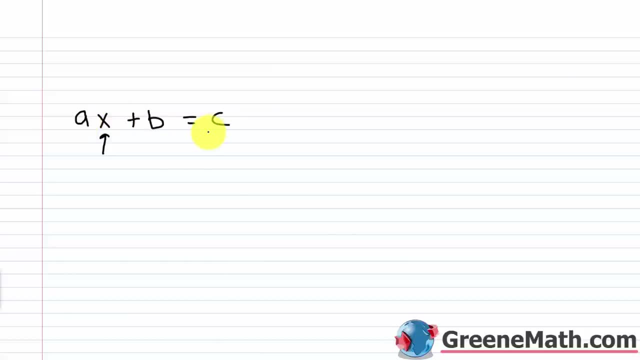 that you could think of. I had one exception to that: Your value for a, which is the coefficient of x, cannot be 0. So a cannot be 0, because, again, if 0 multiplies x, x is going to disappear, right. 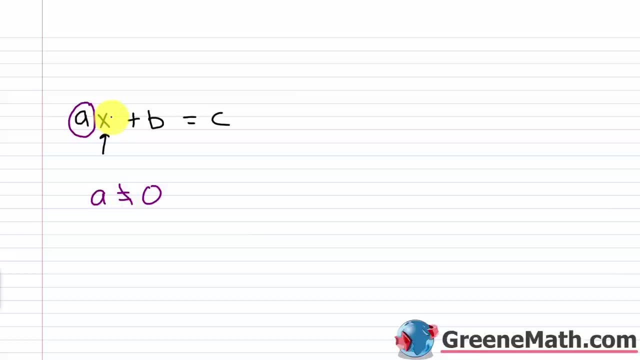 0 times, anything is always 0. So we can't have x dropping out, because this is an equation and we need to have a variable. So, other than that, again, a, b and c can be anything that you want it to be. 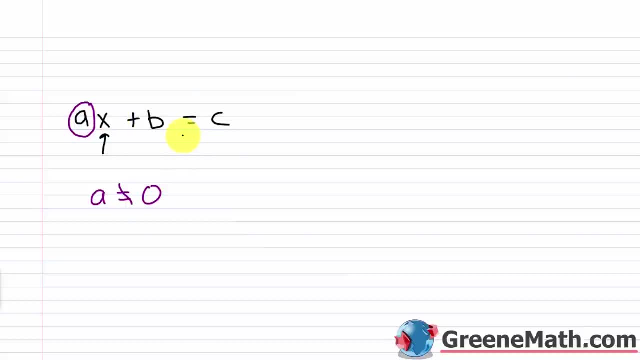 Now, specifically in the last lesson we looked at the case where a was 1, right, We had 1x plus b equals c. 1 times x, anything times 1 is just itself. So really we saw x plus b equals c. 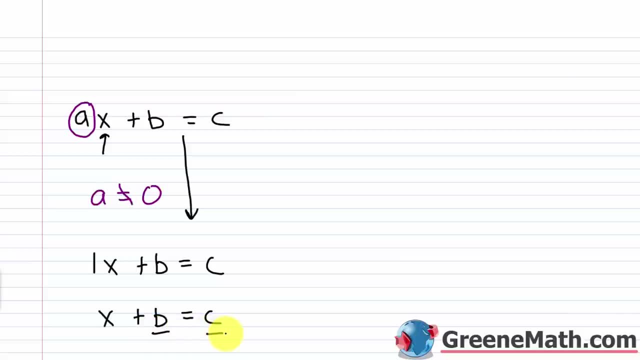 So x plus some number equals some other number. So as an example here we have: x minus 9 equals negative 2.. And I can rewrite this as: x plus negative 9 equals negative 2.. So x plus some number equals some number. 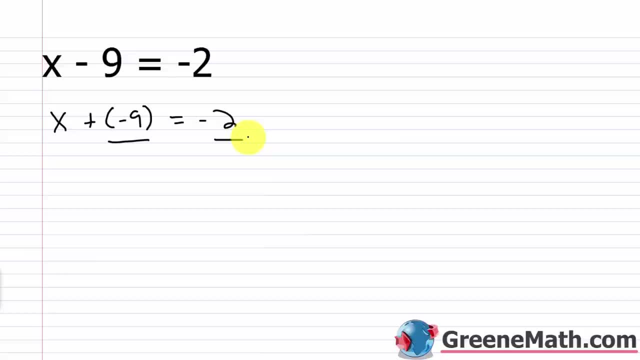 So we learned how to solve an equation of this form. Basically, we do it in one step, using something known as the addition property of equality. The addition property of equality tells us that we can add or also subtract the same number to or, in the case of subtraction. 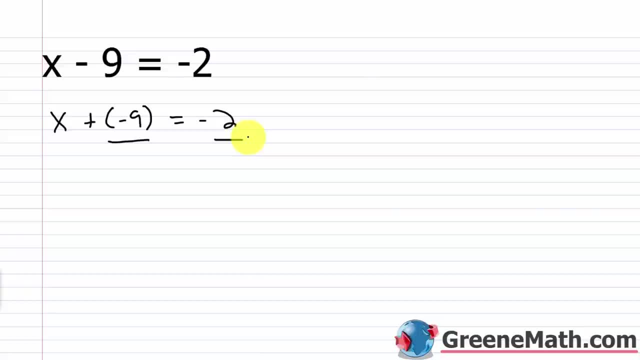 from both sides of an equation without changing the solution, And that's the key. As I go through the steps to solve an equation, I need my solution to stay the same, Because if I get a solution at the end and it doesn't work in the original equation, what use is it? 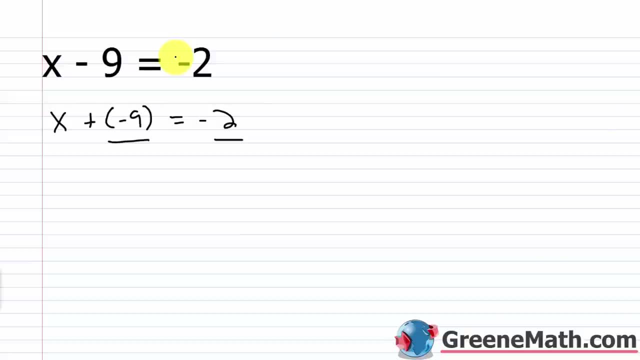 Well, the key is: I can add the same number again to both sides of the equation and it doesn't change the solution. Now, the way we use that, our goal when solving an equation is to isolate the variable. In this case, that would be x. 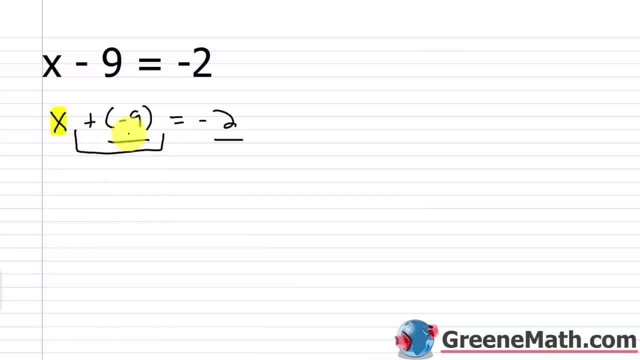 Now, if I look on the left side of the equation, I have this plus negative 9.. I've got to think of a way to get rid of that, because I just want x by itself. I want x equals something, so I can have a solution. 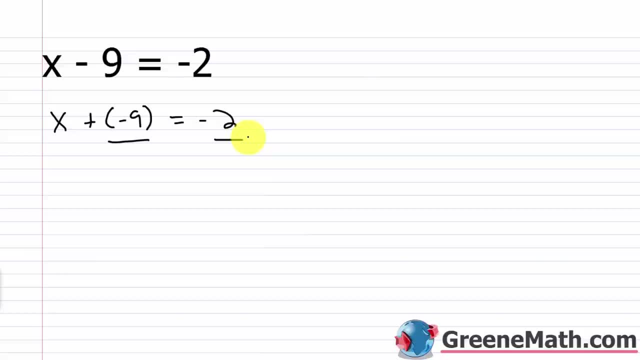 of this form basically we do it in one step using something known as the addition property of equality the addition property of equality tells us that we can add or also subtract the same number two or in the case of subtraction from both sides of an equation without changing the solution and that's the key as i go through the steps to solve an equation i need my solution to stay the same because if i get a solution at the end and it doesn't work in the original equation what use is it so the key is i can add the same number again to both sides of the equation and it doesn't change the solution now the way we use that our goal when solving an equation is to isolate the variable in this case that would be x now if i look on the left side of the equation i have this plus negative nine i've got to think of a way to get rid of that because i just want x by itself i want x equals something so i can have a solution remember that if i add negative nine and positive nine i get zero and if i had x plus zero that would simplify to just x so what i'm going to do is on the left side i'm going to add the opposite of negative 9 which again is positive 9 and because i do that to the left side i must also do it to the right side so i added 9 here and i added 9 here 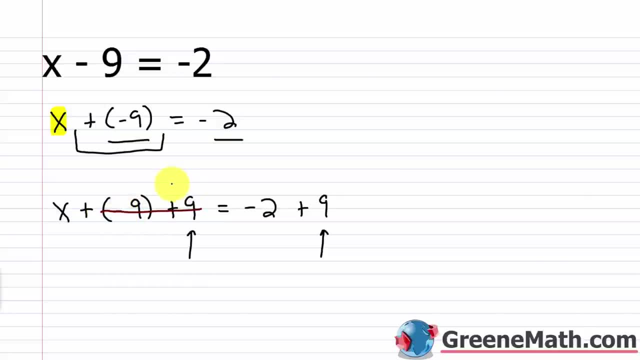 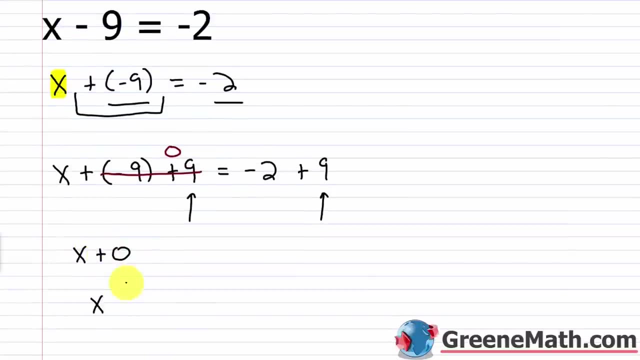 and now on the left side negative 9 plus 9 is 0. so i would have x plus 0 x plus 0 and now on the right side i have negative 2 plus 9 which is 7 and so i'd have x equals 7 as my solution 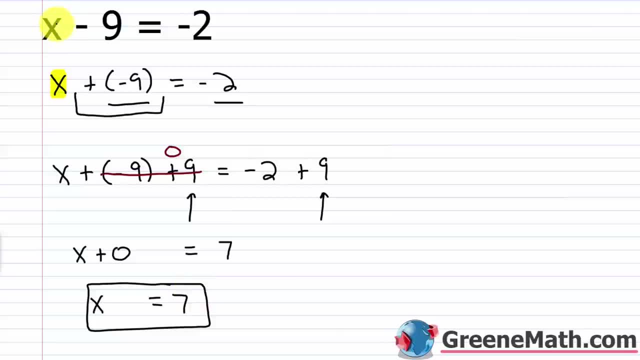 and if you want to you can take a 7 and plug that in for x in the original equation and say 7 minus 9 equals negative 2 and that's true the left side would simplify to negative 2 and the right side is negative 2. so the same value is on both sides of the equation and so we know that this solution x equals 7 is correct 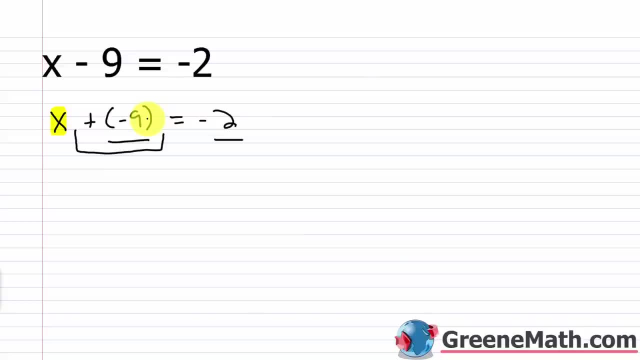 Remember that if I add negative 9 and positive 9, I get 0. And if I had x plus 0, that would simplify to just x. So what I'm going to do is, on the left side, I'm going to add the opposite of negative 9,. 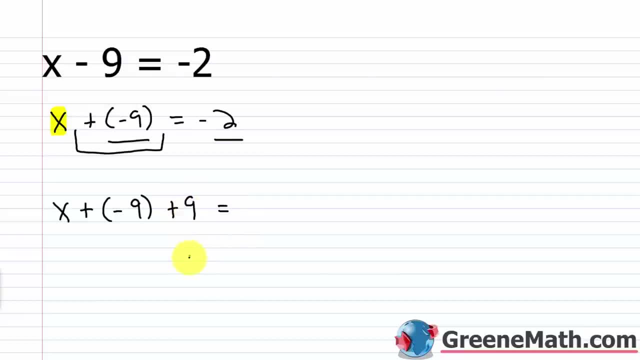 which again is positive 9.. And because I do that to the left side, I must also do it to the right side. So I added 9 here and I added 9 here, And now, on the left side, negative 9 plus 9 is 0.. 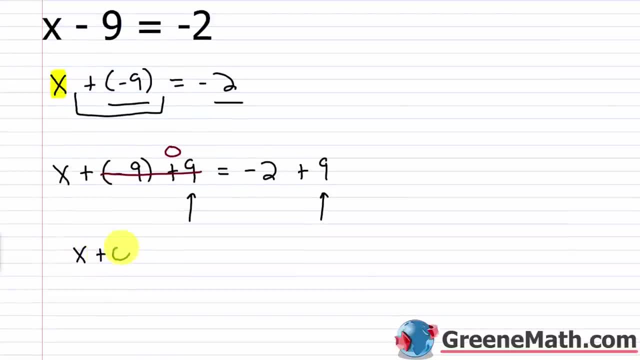 So I would have x plus 0,, x plus 0,, which simplifies to just x. On the right side, I'd have negative 2 plus 9,, which is 7. And so I'd have x equals 7 as my solution. 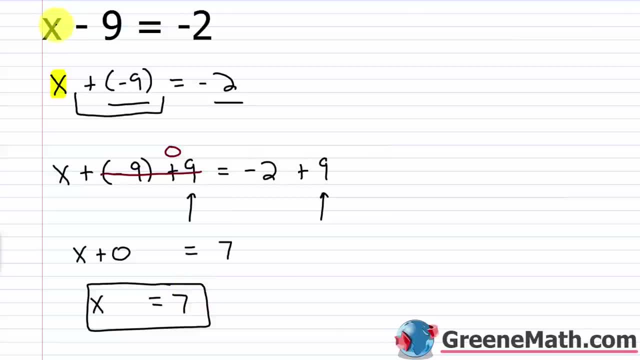 And if you want to, you can take a 7 and plug that in for x in the original equation and say 7 minus 9 equals negative 2. And that's true. The left side would simplify to negative 2, and the right side is negative 2.. 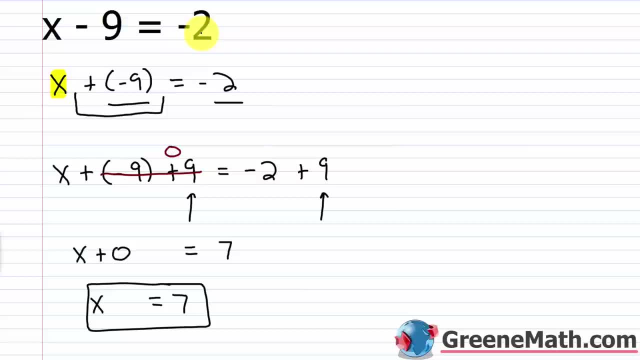 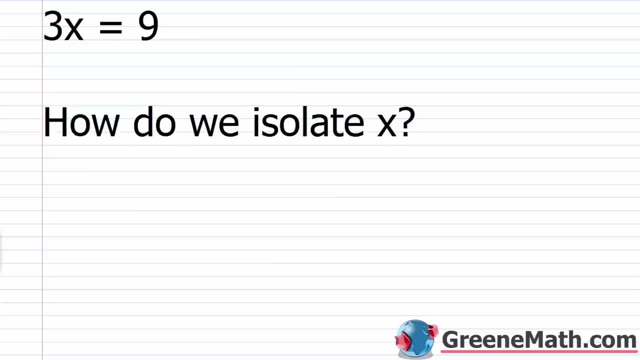 So the same value is on both sides of the equation, And so we know that this solution x equals 7 is correct. Now suppose I give you something like 3x equals 9.. How do we isolate x here? Again, this is our goal: to isolate x. 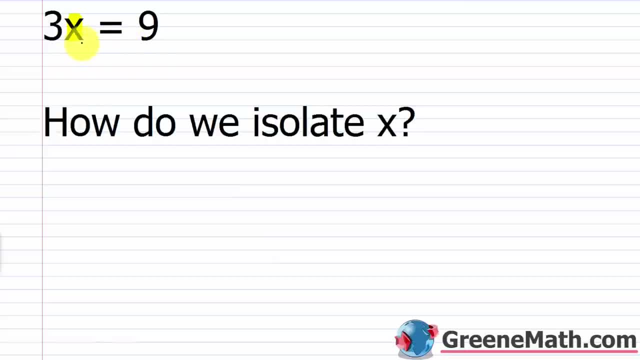 Well, now you'll notice that I don't have anything that's being added to x. Now I have something that's multiplying x. So how do we isolate x in this case? Well, we need to think about a few different properties. first, 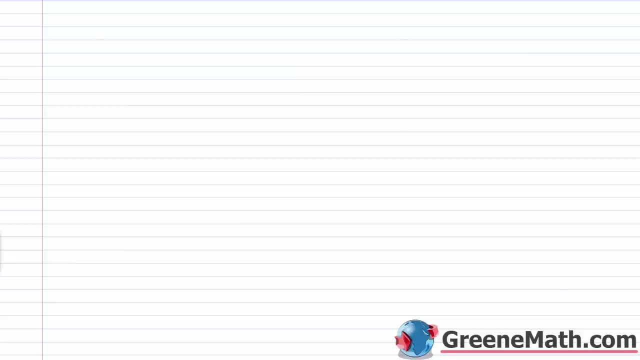 and then we're going to revisit this problem. So the first thing is that a number times its reciprocal is always 1.. So we think about reciprocals when we think about fractions. right, If I have something like 2 fifths? 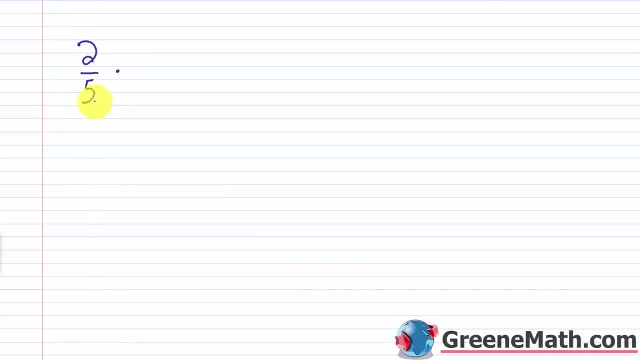 and I multiply by the reciprocal of 2 fifths. remember, I take the denominator and I put it in the numerator, and I take the numerator and put it in the denominator, So a number like 2 fifths times its reciprocal. 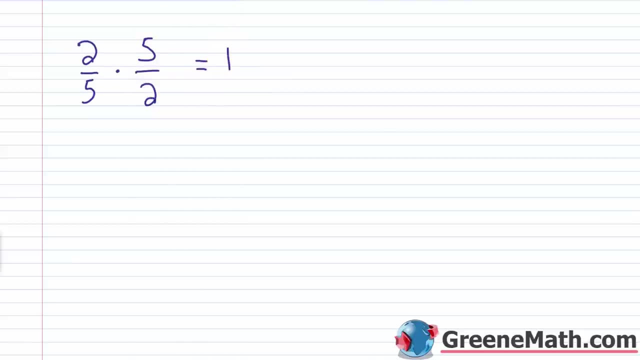 which is 5 halves, will always be 1.. And why is that the case? Well, if I cross cancel, this 5 will cancel with this 5 and give me 1.. This 2 will cancel with this 2 and give me 1.. 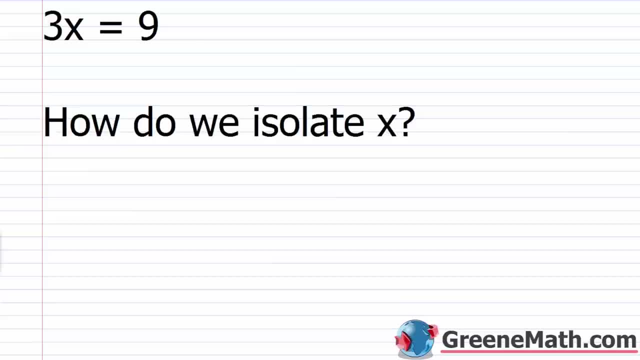 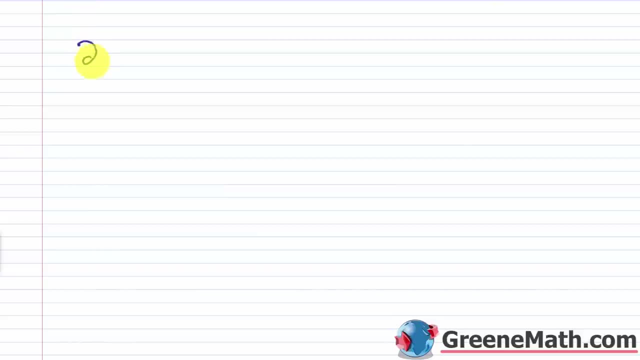 reciprocals when we think about fractions right if i have something like two-fifths and i multiply by the reciprocal of two-fifths remember i take the denominator and i put in the numerator and i take the numerator and put in the denominator so a number like two-fifths times this reciprocal 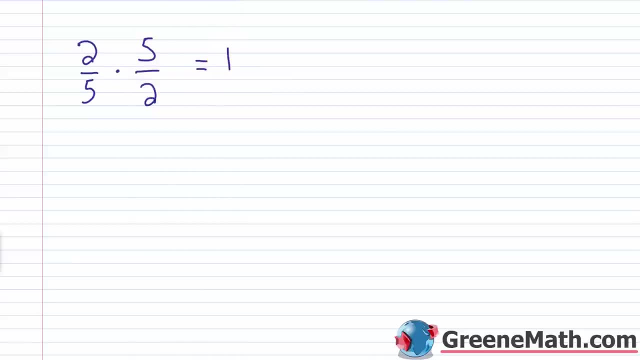 which is five halves will always be one and why is that the case well if i cross cancel this 5 will cancel with this 5 and give me 1 this 2 will cancel with this 2 and give me 1 so i basically have 1 x 1 which equals 1. so i basically have 1 x 1 which equals 1. 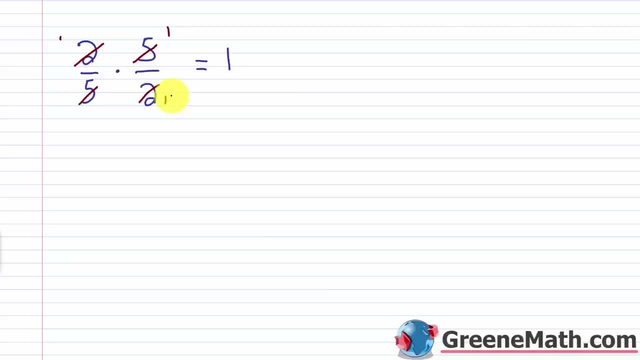 so i basically have 1 x 1 which equals 1. one now this is always true a number times this reciprocal is always one and you can see a kind of more advanced example of that let's say 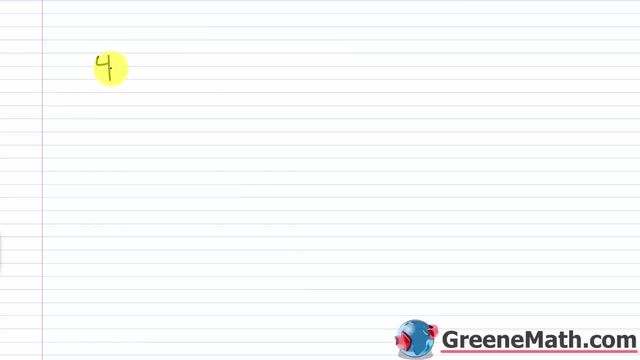 i had the number four what is a reciprocal of four remember you could write four is four over one 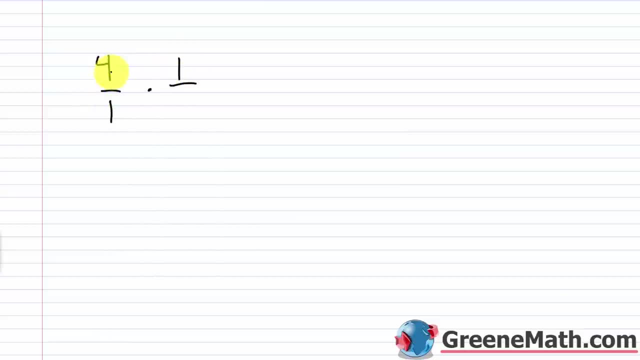 and then the reciprocal would be take one and put it in the numerator take four and put in the denominator and again everything is going to cancel this four is going to cancel with this four 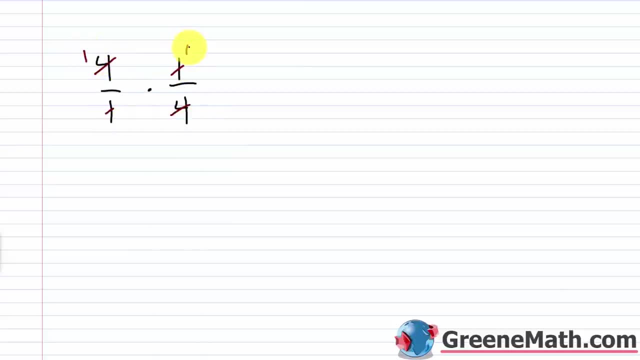 you really think of this one cancelling with this one i mean it's just going to be one so you have 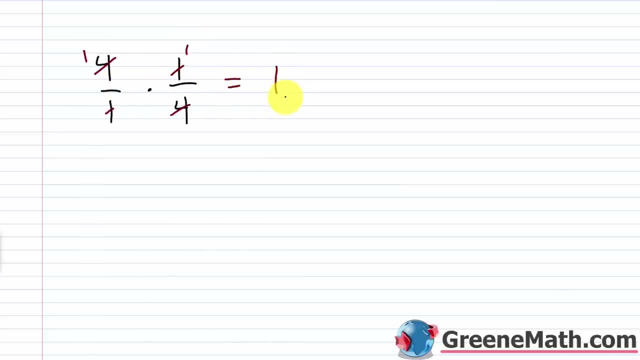 equals 1. So again, a number times its reciprocal is always 1. Alright, another fact that you 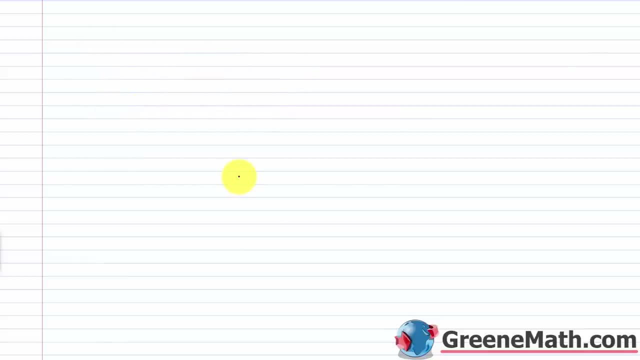 might want to think about is that a non-zero number divided by itself is also always 1. 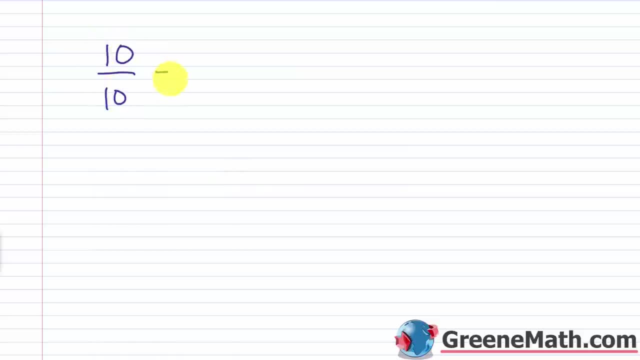 So for example, 10 divided by 10 equals 1. 1037 divided by 1037 is 1. Any non-zero number divided by itself is 1. You have to exclude 0 in that because you can't say 0 divided 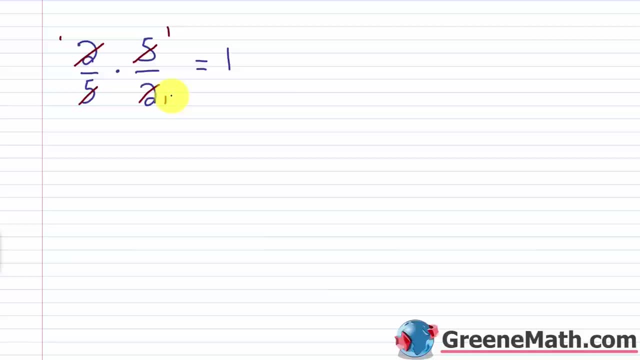 So I basically have 1 times 1,, which equals 1.. Now, this is always true. A number times its reciprocal is always 1.. And you can see a kind of more advanced example of that. Let's say I had the number 4.. 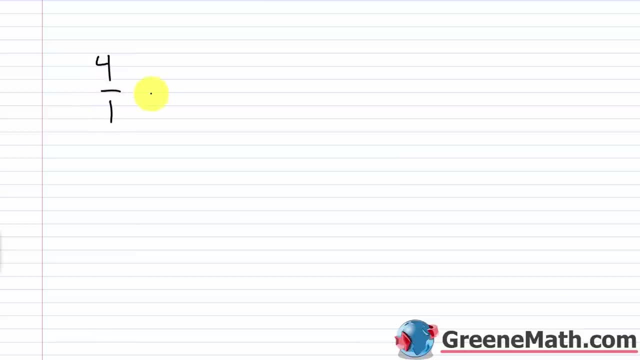 What is a reciprocal of 4?? Remember you could write 4 as 4 over 1, and then the reciprocal would be: take 1 and put it in the numerator, take 4 and put it in the denominator, And again everything's going to cancel. 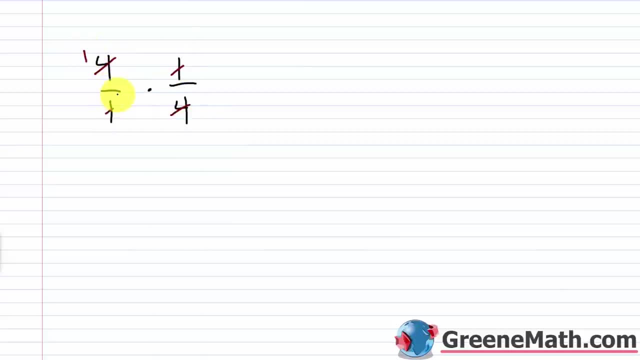 This 4 is going to cancel with this 4.. You really think of this 1 canceling with this 1, I mean it's just going to be 1.. So you have 1 times 1, which equals 1.. 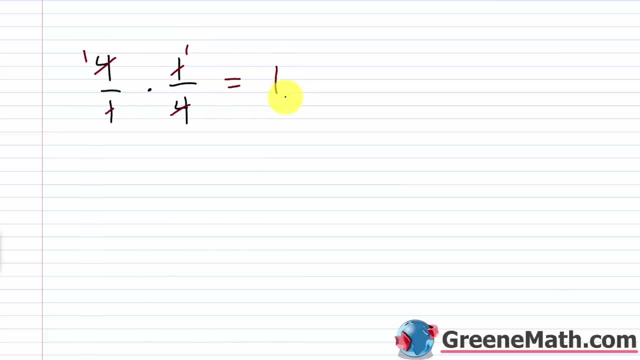 So again a number times: its reciprocal is always 1.. All right, another fact that you might want to think about is that a nonzero number divided by itself is also always 1.. So, for example, 10 divided by 10 equals 1.. 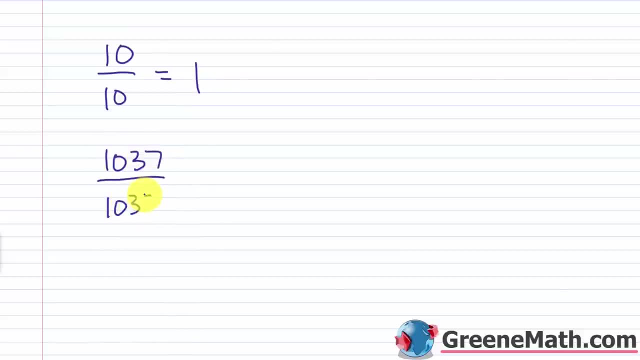 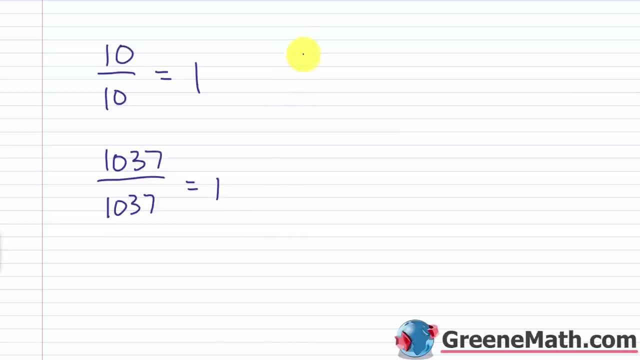 Any nonzero number divided by itself is 1.. You have to exclude 0 in that, because you can't say 0 divided by 0 equals 1, because you can't divide by 0, right 0 can never be in the denominator. 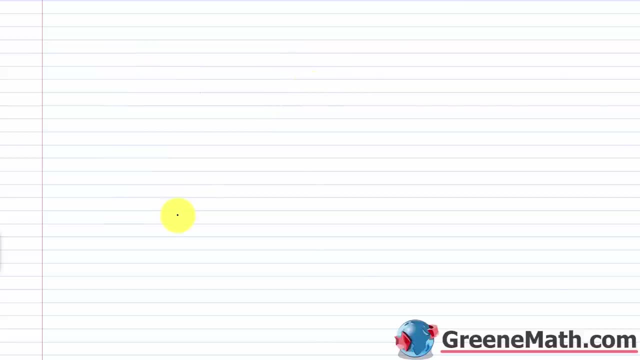 So that's why we say any nonzero number divided by itself is 1.. So then there's one more thing I want you to note, and that's that if you multiply a number by 1, it remains unchanged, So it doesn't matter what it is. 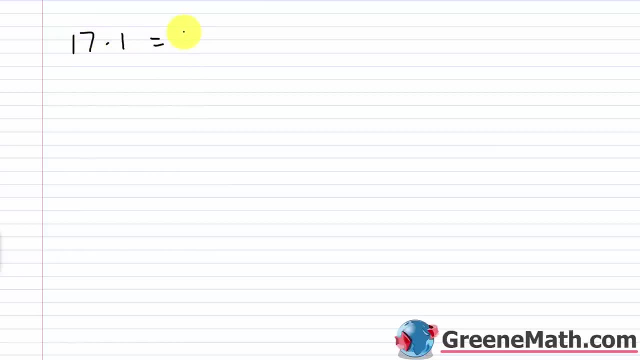 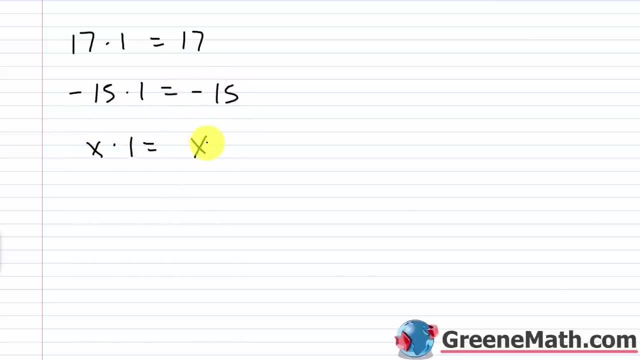 So x times 1 equals x Or z squared times 1 equals z squared. Or if I wrote it a different way and put 1y, that's just equal to y. right, That's just equal to y. 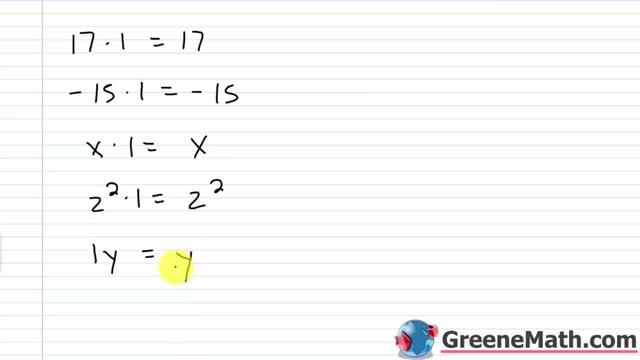 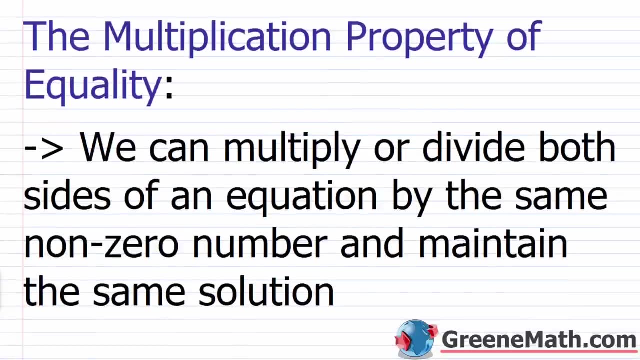 So a lot of times we'll see 1 as the coefficient of a variable and we just write that variable without the 1, right, Because it's the same thing, All right. so now let's talk about the multiplication property of equality. 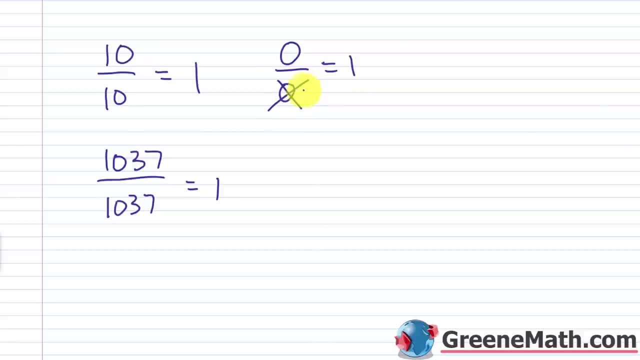 by 0 equals 1 because you can't divide by 0. 0 can never be in the denominator. So that's why we say any non-zero number divided by itself is 1. So then there's one more thing 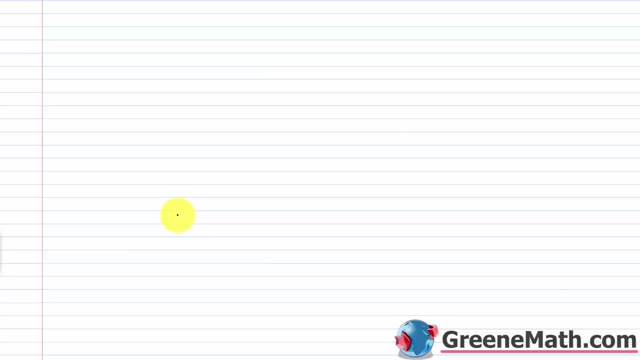 I want you to note, and that's that if you multiply a number by 1, it remains unchanged. So it doesn't matter what it is. So 17 times 1 equals 17. Negative 15 times 1 equals negative 15. 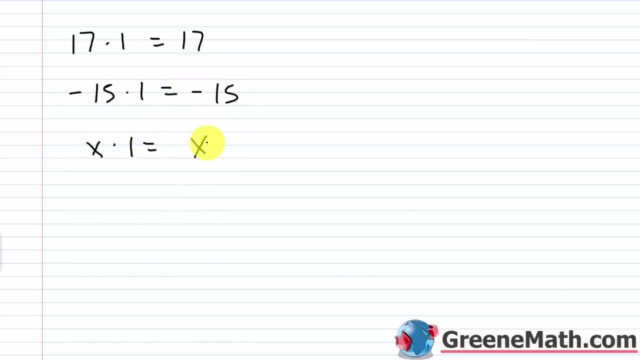 So x times 1 equals x. Or z squared times 1 equals z squared. Or if I wrote it a different way and put 1y, that's just equal to y. So a lot of times we'll see 1 as the coefficient of a variable, and we just write that variable without the 1 because it's the same thing. 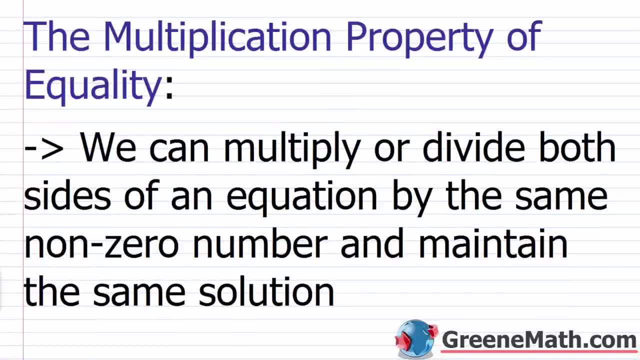 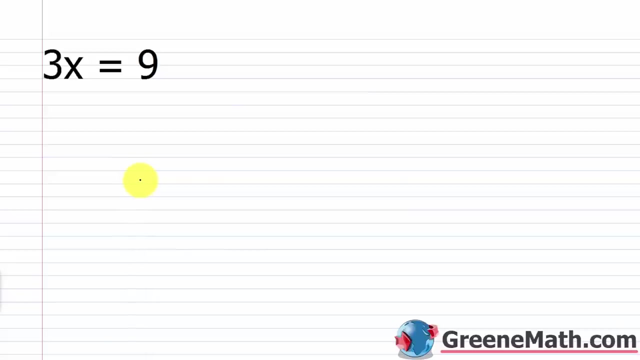 Alright, so now let's talk about the multiplication property of equality. So we can multiply or divide both sides of an equation by the same non-zero number, and that's important. 0 is not involved here, and maintain the same solution. If you use 0 to multiply, remember, if you multiply 0 by something, it becomes 0. So 0 is not going to work for our multiplication property of equality. It has to be the same non-zero number. Alright, so let's revisit our 3x equals 9. So again, our goal is to isolate the variable from the equation, and we're going to do that by dividing both sides of an equation by the same non-zero number. So we want to isolate this. And what can we do to get x by itself? Well, I have 3 multiplied by x equals 9. I want you to think back to what I just said a minute ago. A number divided by itself is 1. So if I divided, if I divided the left side here by the coefficient of x, which is 3. 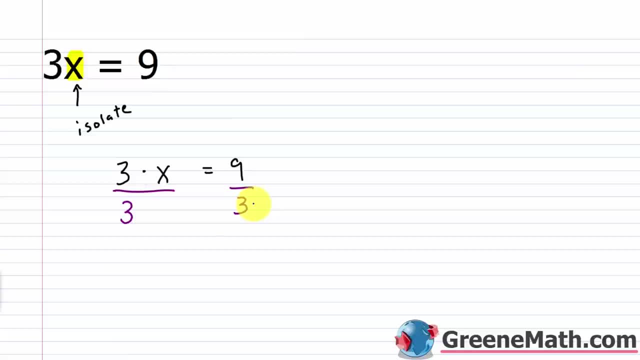 I would have x by 3. And to make it legal, divided this by 3. What would happen over here is I would have 3 divided by 3, which is 1. And then 1 times x would just be x. 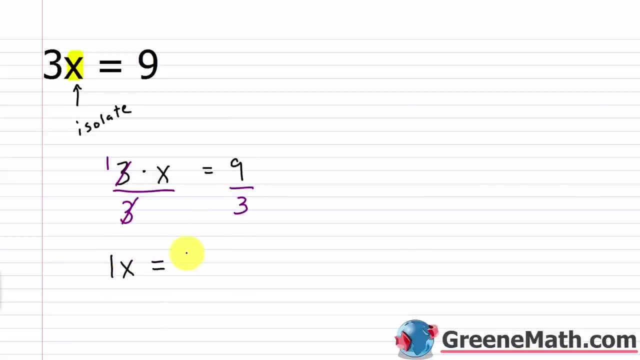 Alright, this would be 1x equals, 9 divided by 3 is 3. 1x equals 3, or x equals 3. So 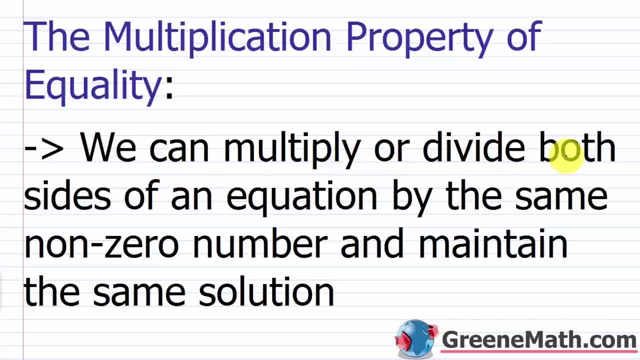 So we can multiply a number by 1.. So we can multiply or divide both sides of an equation by the same non-zero number- and that's important, Zero is not involved here- And maintain the same solution If you use zero to multiply, remember if you multiply zero by something, it becomes zero. 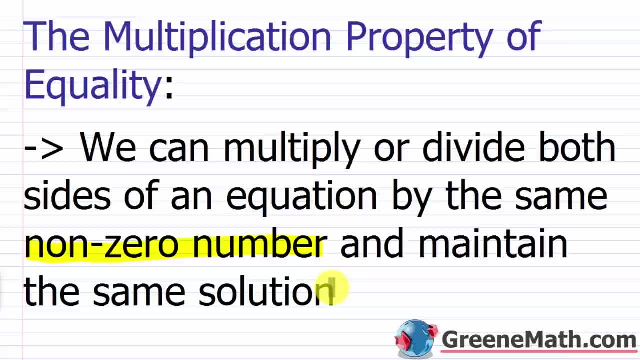 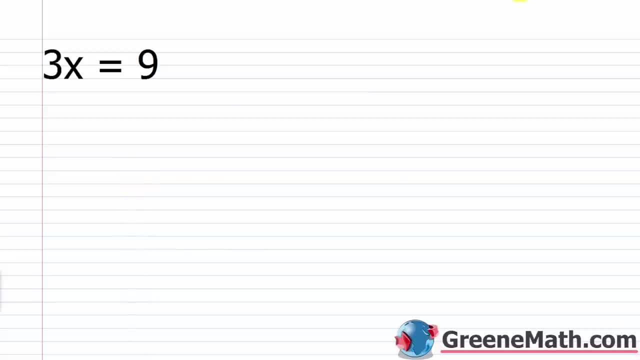 So zero is not going to work for our multiplication property of equality. It has to be the same non-zero number, All right, so let's revisit our 3x equals 9.. So again, our goal is to multiply by 1.. 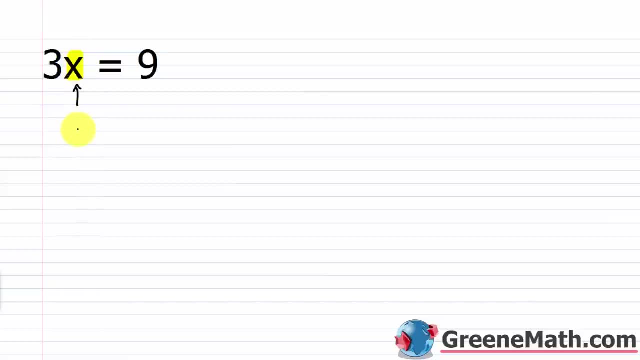 So again, our goal is to multiply by 1.. Our goal is to isolate the variable x. So we want to isolate this. And what can we do to get x by itself? Well, I have 3 multiplied by x equals 9.. 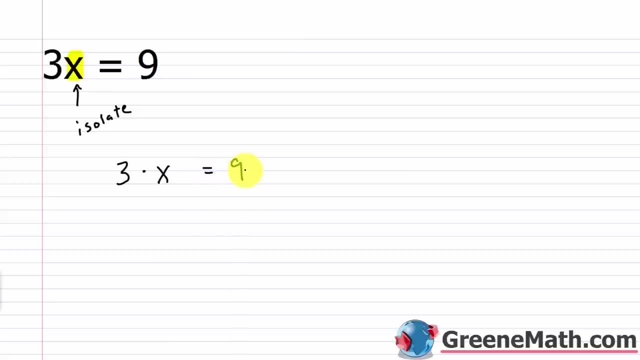 I want you to think back to what I just said a minute ago. A number divided by itself is 1.. So if I divided the left side here by the coefficient of x, which is 3,, if I divided this by 3, and to make it legal, divided this by 3,. 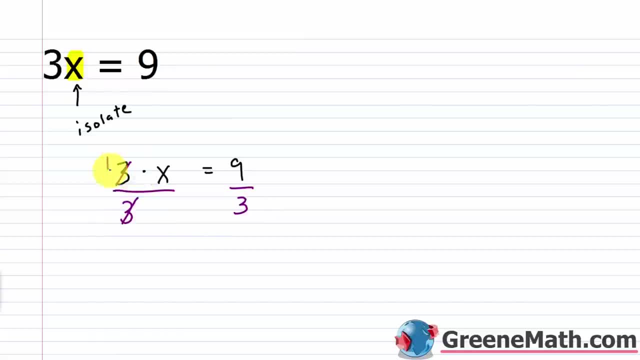 what would happen over here is I would have 3 divided by 3, which is 1, and then 1 times x would just be x. All right, this would be: 1x equals 9, divided by 3 is 3.. 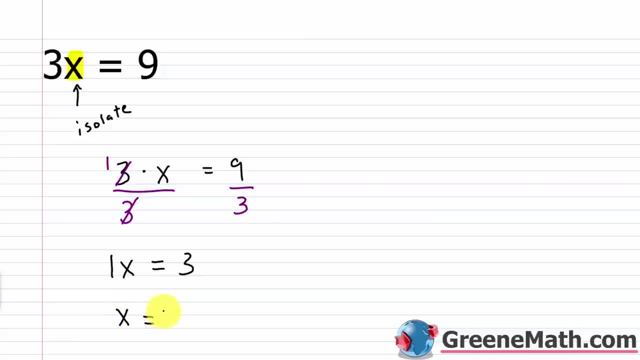 1x equals 3, or x equals 3.. So when you have a number, as we call it, a coefficient, that is multiplying a variable in this format, all you need to do to isolate the variable is divide both sides of the x. 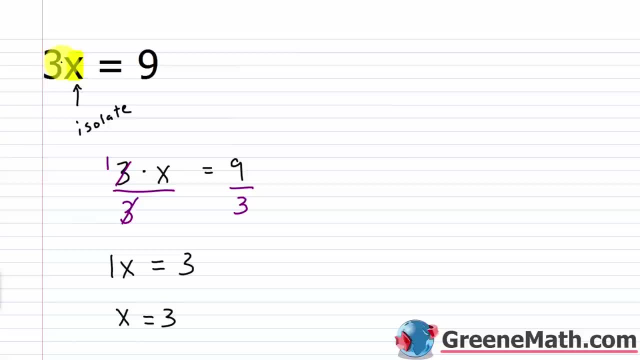 the equation by that number right, by the coefficient of your variable. Another way you can think about this is: I could think of 3 as 3 over 1.. Let's say I had 3 over 1 times x equals 9.. 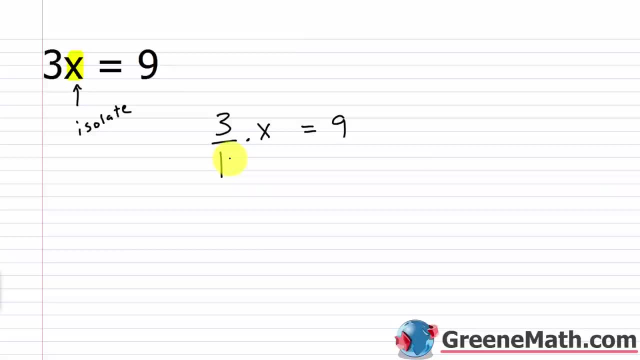 So if I have 3 over 1, again a number times, its reciprocal is always going to be 1.. So I could have also said: okay, I'm going to multiply this side by the reciprocal of 3 over 1.. 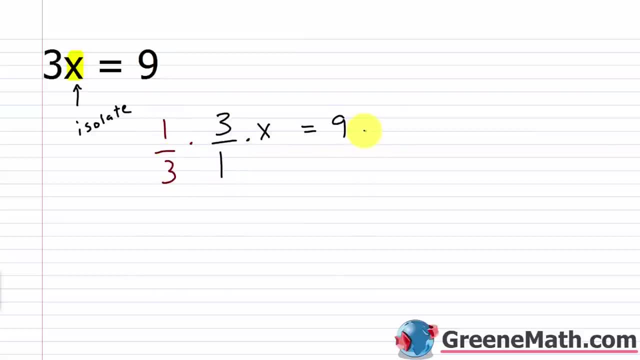 The reciprocal of 3 over 1 is 1 over 3, or 1 third, And I'm going to multiply this by 1 third And you can see that multiplying by a third and dividing by 3, that's the exact same thing. 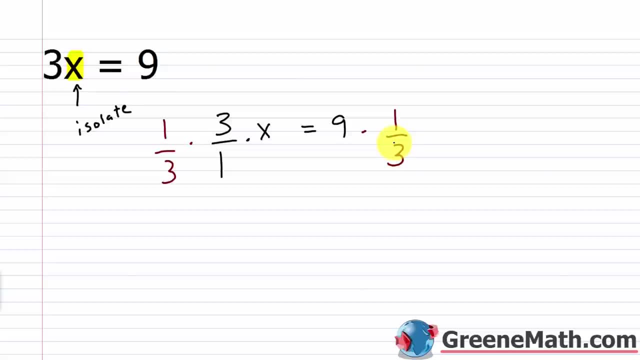 If I multiply by a fourth or I divide by 4, that's the same. If I multiply by a fifth or I divide by 5, that's the same. So what we get here is this: 3 cancels with this 3,. 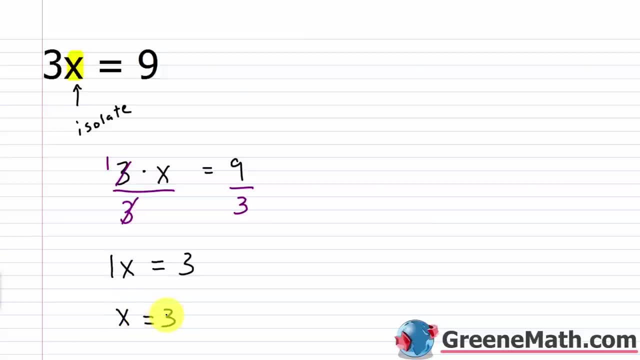 when you have a number, as we call it a coefficient, that is multiplying a variable in this format, all you need to do to isolate the variable is divide both sides of the equation by that number, right, by the coefficient of your variable. Another way you can think about this is, I could think of 3 as 3 over 1. Let's say I had 3 over 1 times x equals 9. So if I have 3 over 1, again, a number times its reciprocal is always going to be 1. So I could have also said, okay, I'm going to multiply this side by the reciprocal of 3 over 1. The reciprocal of 3 over 1 is 1 over 3, or 1 third. And I'm going to multiply this by 1 third. 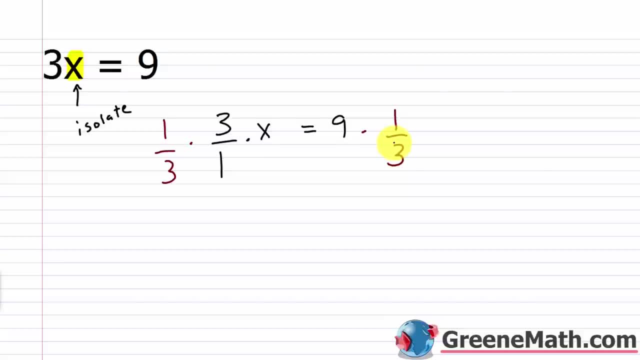 And you can see that. . . . . . . . . . . . . . . . . . . . . . . . . . . . . . . . . . . . . . . multiplying by a third and dividing by 3, that's the exact same thing. If I multiply by a fourth, or I divide by 4, that's the same. If I multiply by a fifth, or I divide by 5, that's the same. So what we get here is this three cancels with this 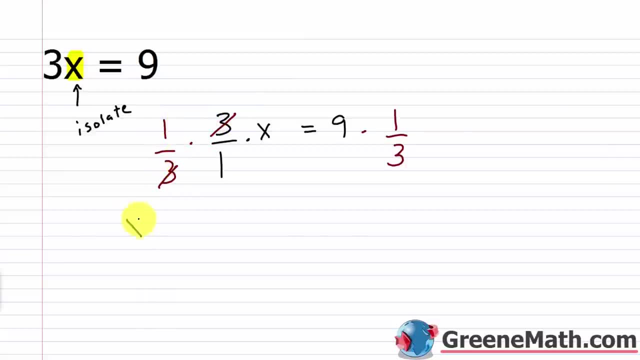 three, and I'll basically have 1 times x, or just x equals this 9 will cancel with this 3 and give me a 3, 3 times 1 is 3, so x equals 3. And again, we always want to check our solution. We might have made a mistake somewhere. 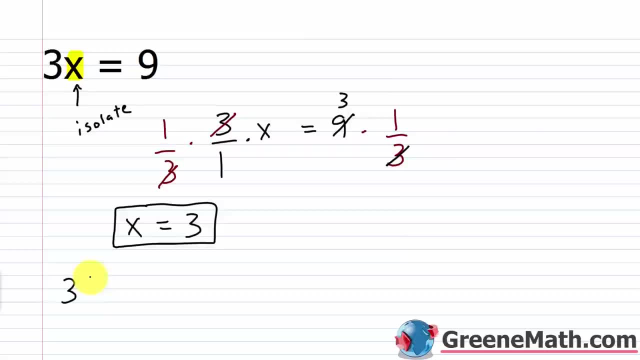 So take the 3 and plug it back in for x. You'd have 3 times 3 is equal to 9. 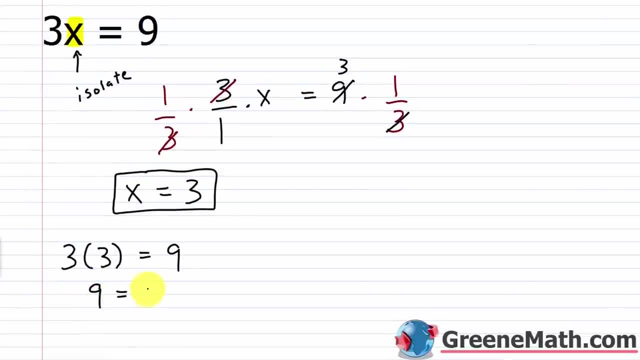 And then over here on the left, 3 times 3 is 9, so you get 9 equals 9. Same value on the left as the right. 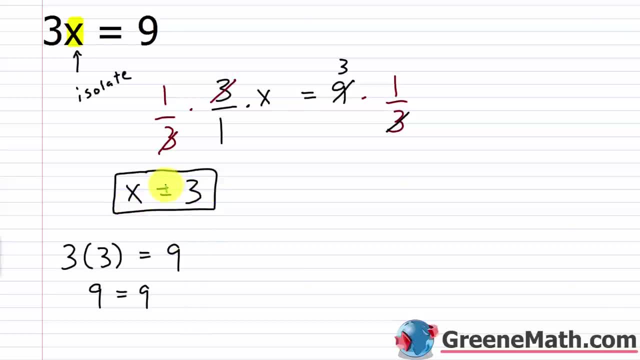 So yeah, we can say that our solution here, x equals 3, is correct. All right, what about 2 thirds x equals 10? 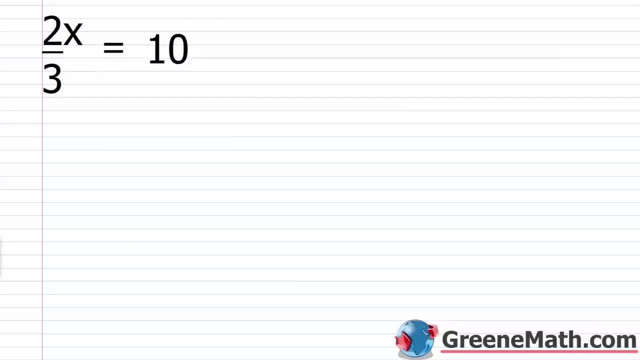 So the coefficient of x, what's multiplying x here is 2 thirds. So how do I isolate x in that scenario? Well again, if I want to get x by itself, one thing I can do is I can multiply both sides by 3 halves. That's the reciprocal of 2 thirds. Remember, if I have 2 thirds and I multiply this by 3 halves, that's going to become 1. 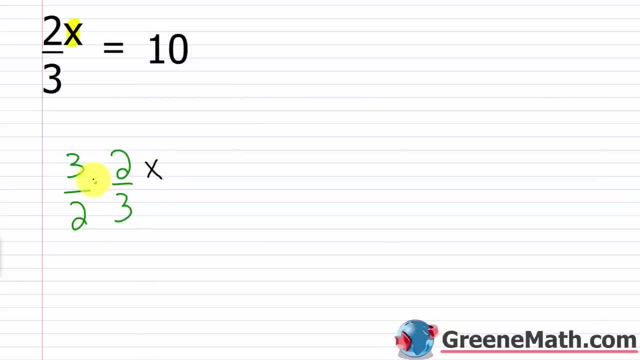 Now the only other thing over here is x, so times x. So this is going to cancel with this and give me 1. This is going to cancel with this and give me 1. So I'll have 1 times x, or just x. Or you can write 1x if you want, and then simplify that just to x. It doesn't really matter. 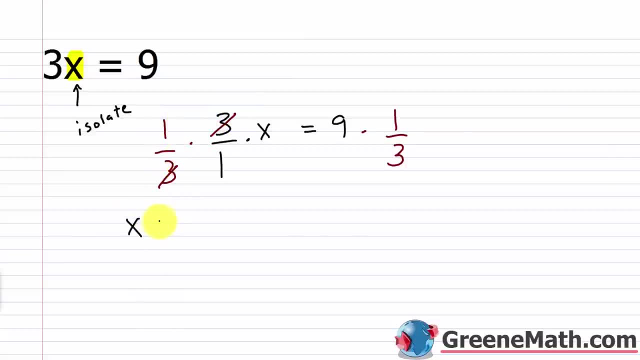 and I'll basically have 1 times x, or just x equals this. 9, will cancel with this 3 and give me a 3.. 3 times 1 is 3.. So x equals 3.. And again, we always want to check our solution. 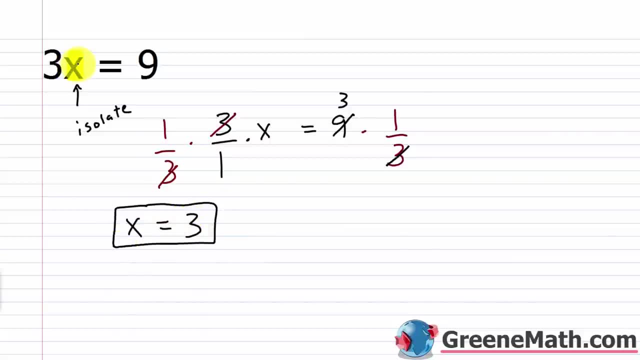 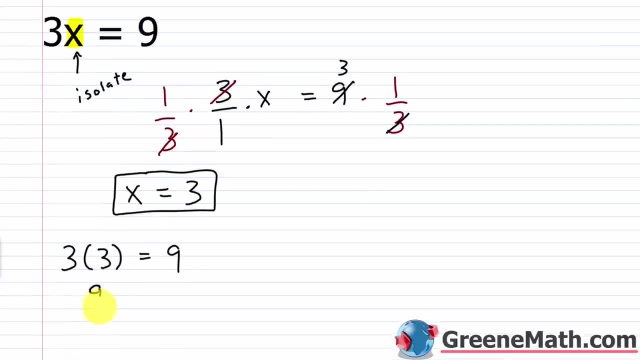 We might have made a mistake somewhere. So take the 3 and plug it back in for x You'd have: 3 times 3 is equal to 9.. And then over here on the left, 3 times 3 is 9, so you get 9 equals 9.. 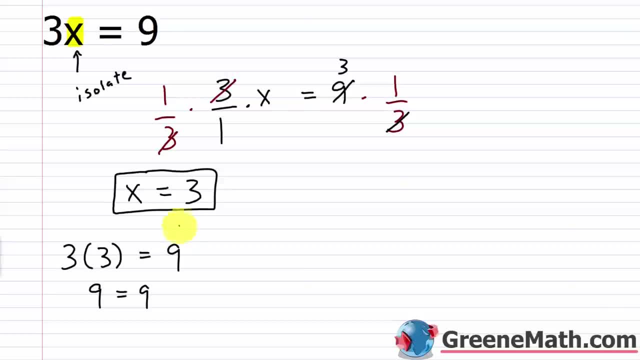 Same value on the left as the right. So yeah, we can say that our solution here- x equals 3, is correct. All right, what about 2 thirds? x equals 10? So the coefficient of x, what's multiplying x? here is 2 thirds. 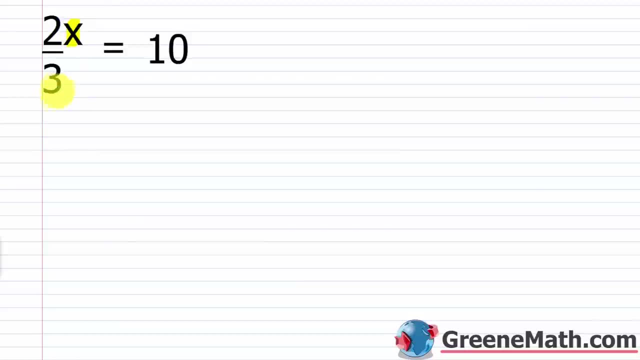 So how do I isolate x in that scenario? Well, again, if I want to get x by itself, one thing I can do is I can multiply both sides by 3 halves. That's the reciprocal of 2 thirds. Remember, if I have 2 thirds and I multiply this by 3 halves, 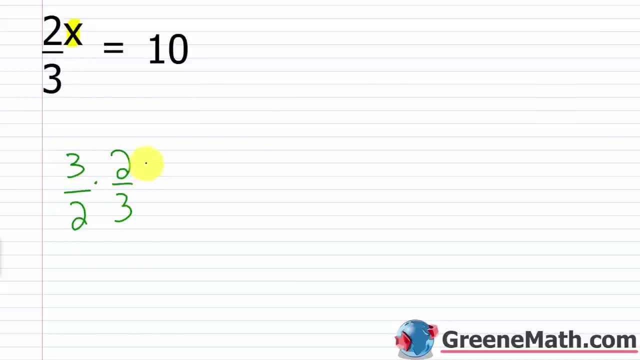 that's going to become 1.. Now, the only other thing over here is x, so times x. So this is going to cancel with this and give me 1.. This is going to cancel with this and give me 1.. 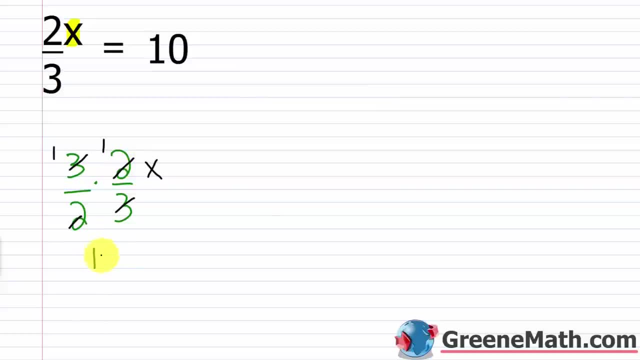 So I'll have 1 times x or just x, Or you can write 1x if you want and then simplify that just to x. Okay, It doesn't really matter, But over here I've got to make sure that because I multiplied by 3 halves. 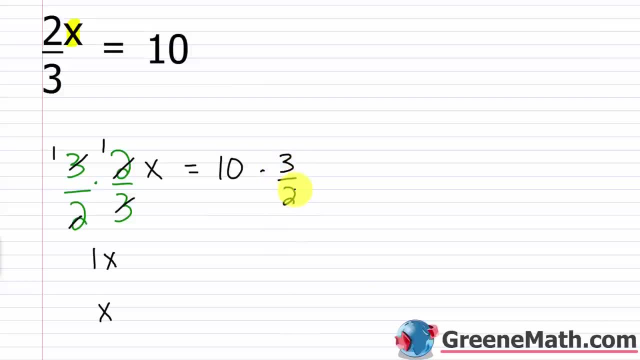 on the left side. I do it to the right side, Otherwise you won't get the correct answer. So 10 times 3 halves This. 10 would cancel with the 2 and give me a 5.. 5 times 3 is 15.. 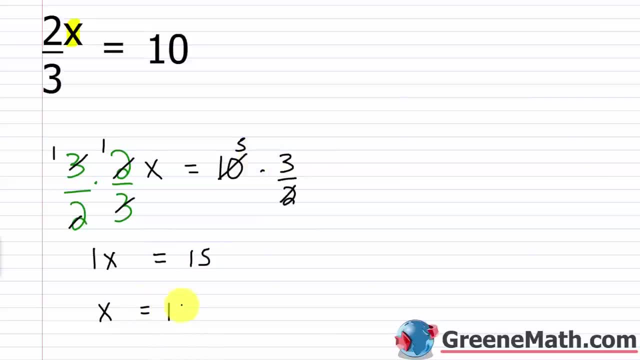 So 1x equals 15.. Again, this will simplify to x equals 15.. So let's check this: x equals 15 real quick. So I'm plugging a 15 in there And I'd have 2 thirds times 15 equals 10.. 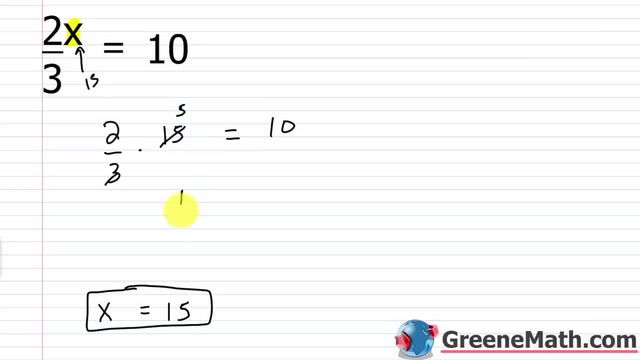 So this 15 would cancel with this 3 and give me a 5.. 5 times 2 is 10.. So I'd get 10 equals 10. Again, the same value on the left as the right. So x equals 15 is correct. 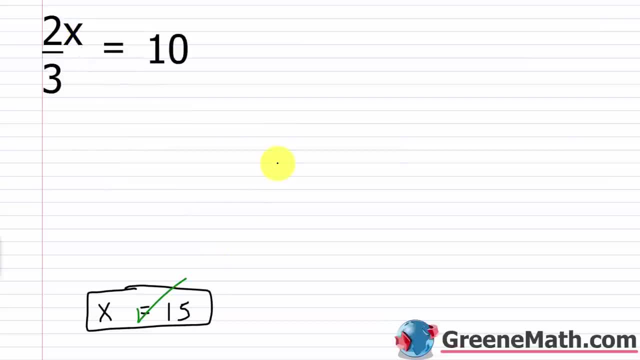 So one thing I just want to bring your attention to: when you're in your textbook on this section about the multiplication property of equality, you basically have two different scenarios. You have a fractional coefficient for x, So like this one: 2 thirds. 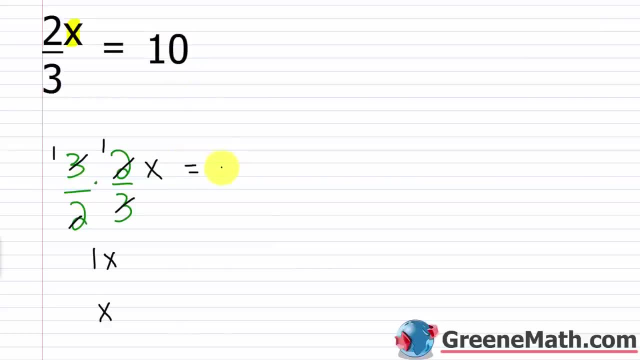 But over here, I've got to make sure that because I multiplied by 3 halves, on the left side, I do it to the right side. Otherwise, you won't get the correct answer. 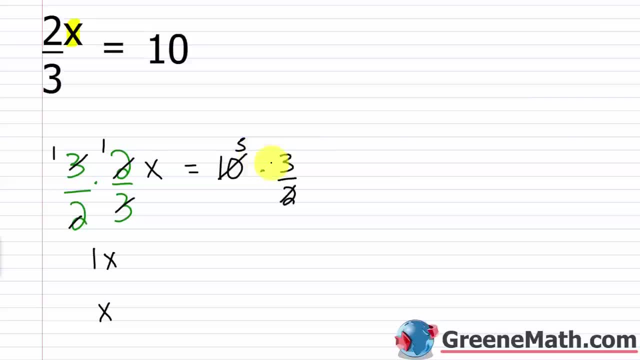 So 10 times 3 halves. This 10 would cancel with the 2 and give me a 5. 5 times 3 is 15. So 1x equals 15. And again, this will simplify to x equals 15. 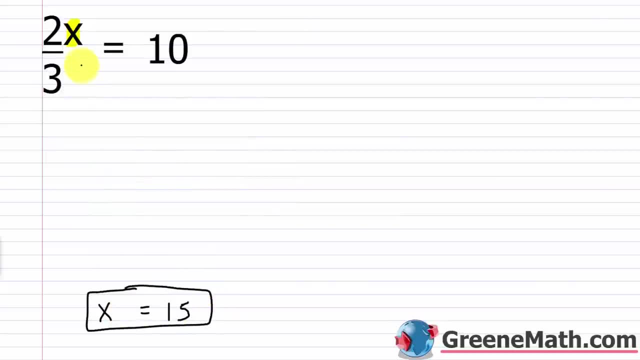 So let's check this x equals 15 real quick. So I'm plugging a 15 in there. And I have 2 thirds. So 1x times 15 equals 10. 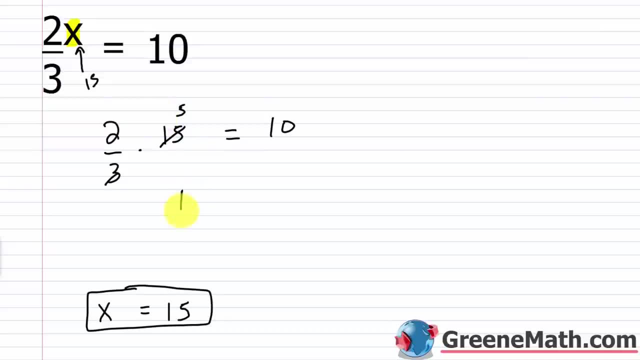 So this 15 would cancel with this 3 and give me a 5. 5 times 2 is 10. So I'd get 10 equals 10. 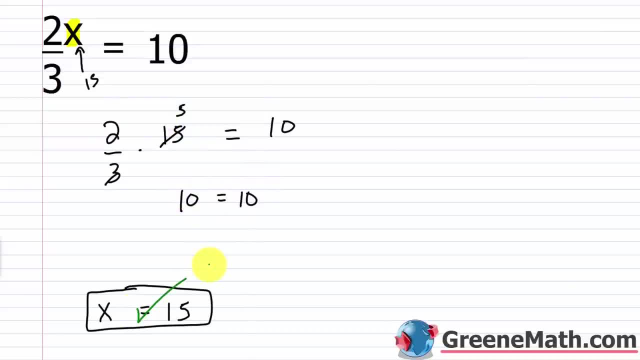 Again, the same value on the left as the right. So x equals 15 is correct. 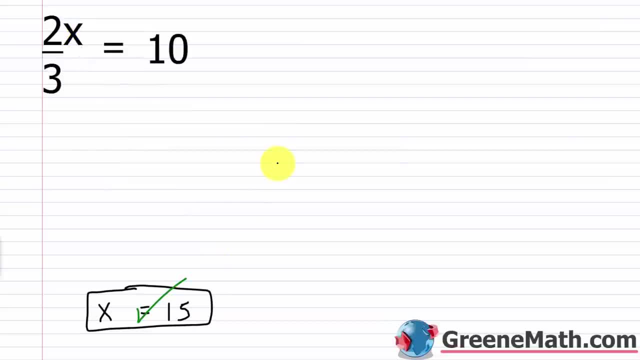 So one thing I just want to bring your attention to, when you're in your textbook on this section about the multiplication property of equality, you basically have two different scenarios. You have a fractional coefficient for x. 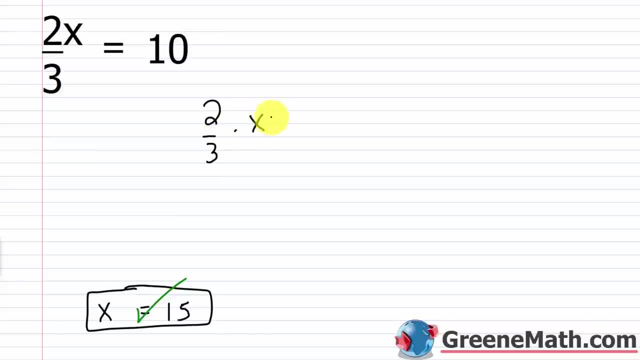 So like this one, 2 thirds times x equals 10. So you have a fractional coefficient for x. So like this one, 2 thirds times x equals 10. So like this one, 2 thirds times x equals 10. So like this one, 2 thirds times x equals 10. 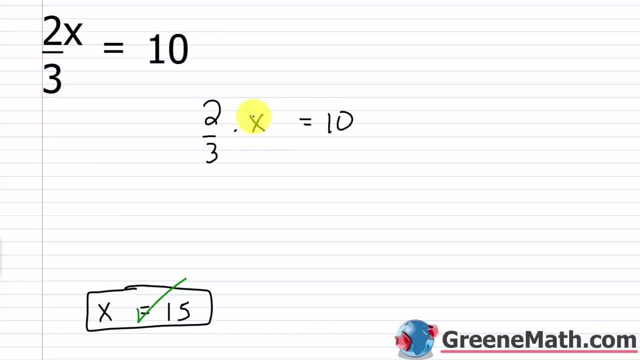 And I'm just writing this out like this just for us to be able to visually see what's going on. And I'm just writing this out like this just for us to be able to visually see what's going on. 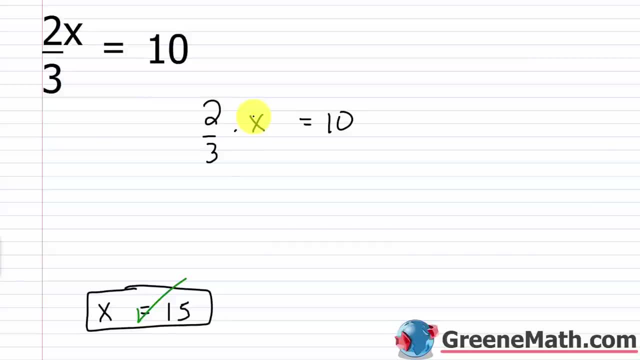 When you have a fractional coefficient, it's going to be faster for you to multiply both sides by the reciprocal of that fraction. 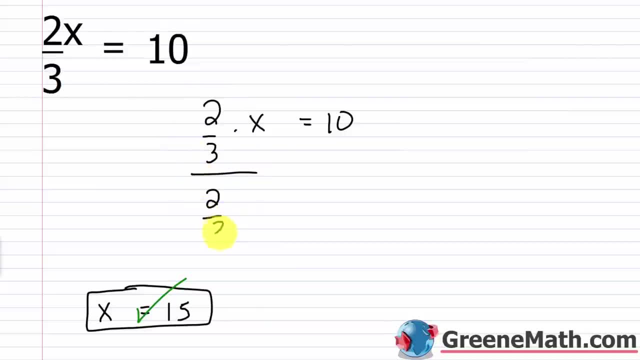 If I wanted to, I could divide both sides by 2 thirds. I can divide both sides by the coefficient of x. I can always do that. So if I divide 2 thirds by 2 thirds, that's going to be what? 2 thirds divided by 2 thirds. The first fraction stays the same. The second fraction, we take the reciprocal. That's 3 halves. And we multiply. Remember, we did that before. We multiplied by 3 halves. 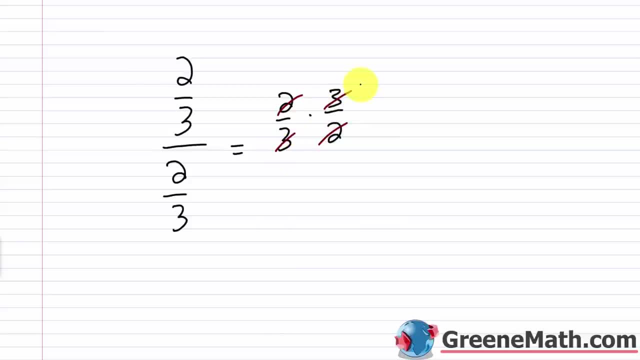 So I'm kind of saving time because this cancels, this cancels. This becomes 1. So we see that this would become 1. So you just have x on this side. 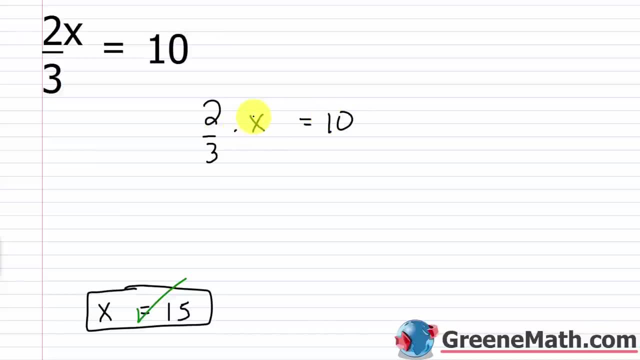 times x equals 10.. And I'm just writing this out like this just for us to be able to visually see what's going on. When you have a fractional coefficient, it's going to be faster for you to multiply both sides by the reciprocal of that fraction. 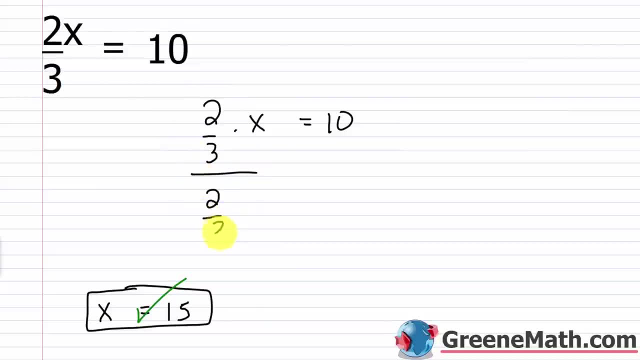 If I wanted to, I could divide both sides by 2 thirds. I can divide both sides by the coefficient of x. I can always do that. So if I divide 2 thirds by 2 thirds, that's going to be what. 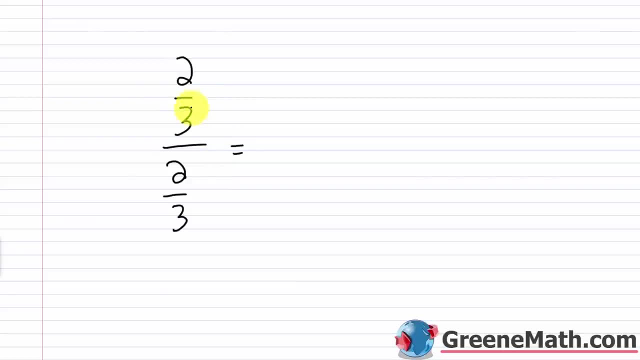 2 thirds divided by 2 thirds, The first fraction stays the same. The second fraction, we take the reciprocal, that's 3 halves, and we multiply. Remember we did that before. We multiplied by 3 halves. So I'm kind of saving time because this cancels, this cancels right. 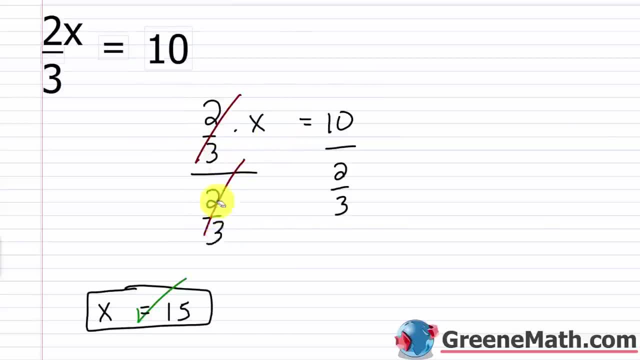 This becomes 1.. So we see that this would become 1, right, So you just have x on this side Now over here. 10 divided by 2 thirds. So 10 divided by 2 thirds. 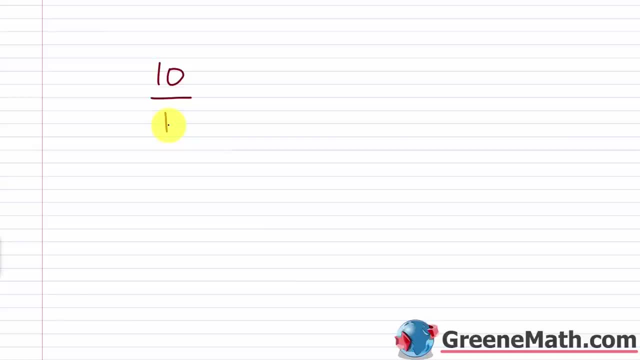 And remember the way we do. that is, we write 10 as 10 over 1. And we multiply by the reciprocal of 2 thirds, which is 3 halves. Again, that's what I did. So this cancels with this and becomes 5.. 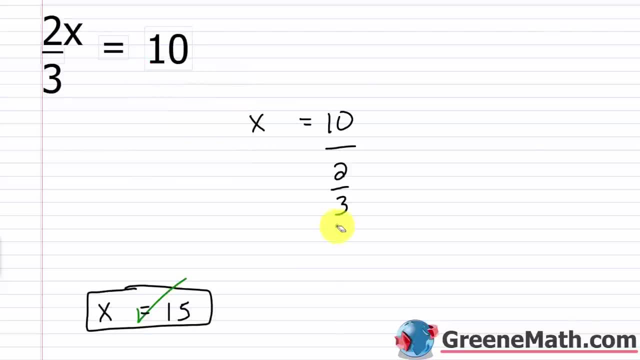 5 times 3 is 15.. So this simplifies to 15 over here And we got that by just multiplying both sides by the reciprocal. so it was kind of like a faster way than doing the division right, Because you got to go through and kind of set things up. 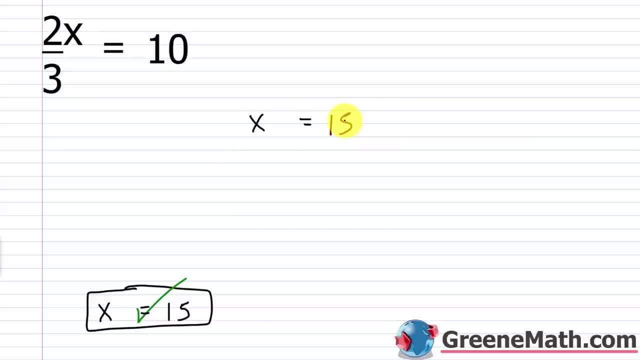 So if you see a fractional coefficient for x, you want to multiply both sides by the reciprocal of that fractional coefficient. If you don't have that, if you have, for example, an integer coefficient, let's say it's negative 2.. 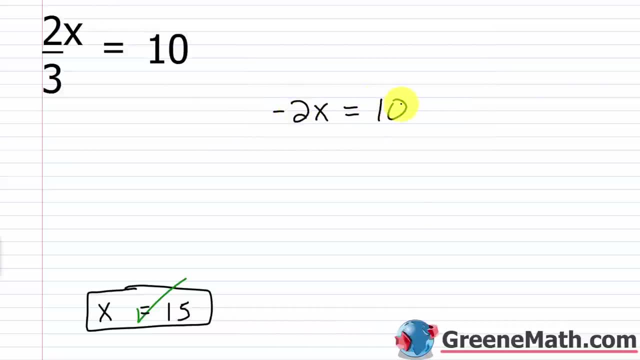 So let's say I have negative 2x equals 10, for example. Well, in this case, yeah, I can go through and multiply by the reciprocal. The reciprocal of negative 2 is negative 1, half. I can do that. 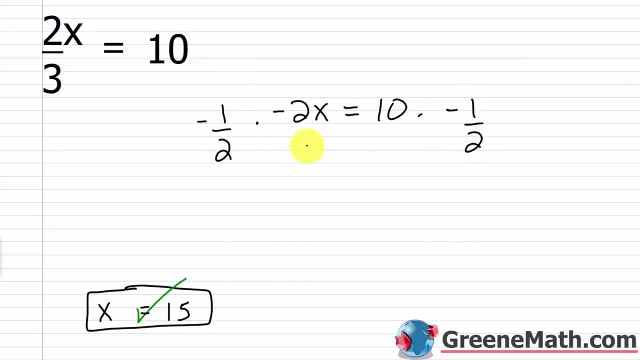 But really it's kind of just faster just to divide in this scenario, right? So in this scenario I wouldn't do that. I would just say: okay, the coefficient of x is negative 2. So to get x by itself, I would divide both sides. 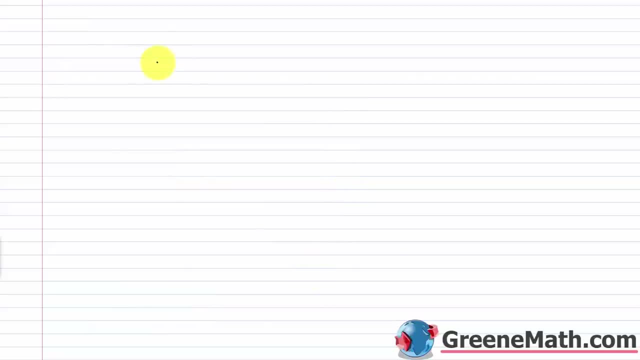 Now, over here, 10 divided by 2 thirds. So 10 divided by 2 thirds. And remember, the way we do that is we write 10 as 10 over 1. 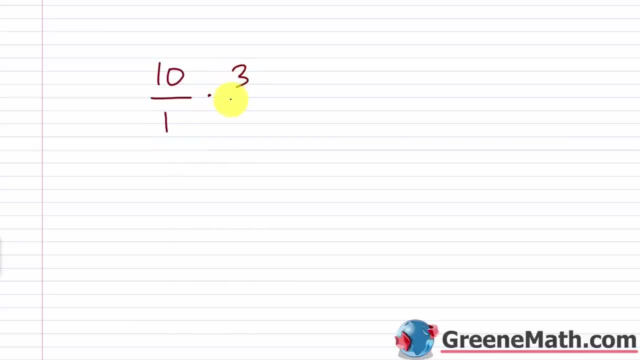 And we multiply by the reciprocal of 2 thirds, which is 3 halves. Again, that's what I did. So this cancels with this and becomes 5. 5 times 3 is 15. So this simplifies to 15 over here. And we got that by just multiplying both sides by the reciprocal. So it was kind of like a faster way than doing the division, right? Because you've got to go through and kind of set things up. 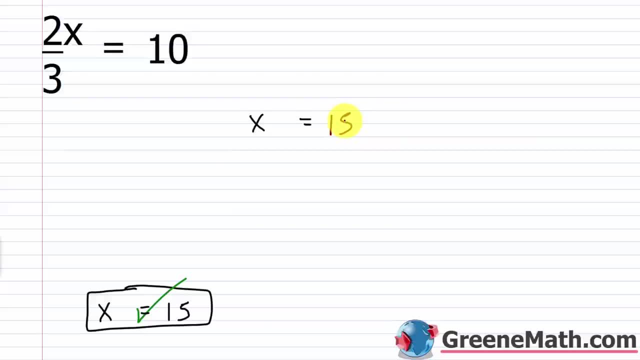 So if you see a fractional coefficient for x, you want to multiply both sides by the reciprocal. 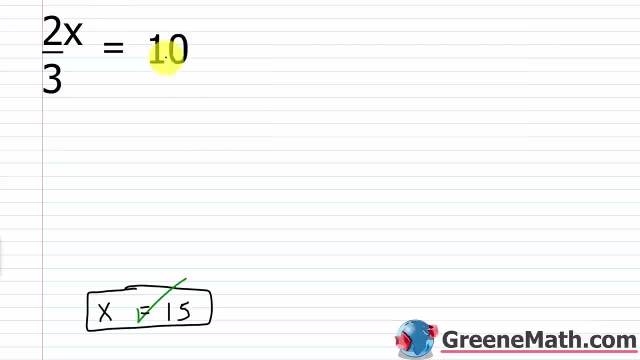 If you don't have that, if you have, for example, an integer coefficient, let's say it's negative 2. So let's say I have negative 2x equals 10, for example. 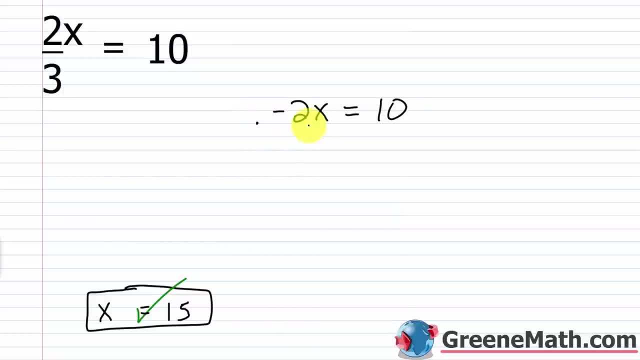 Well, in this case, yeah, I can go through and multiply by the reciprocal. The reciprocal of negative 2 is negative 1 half. 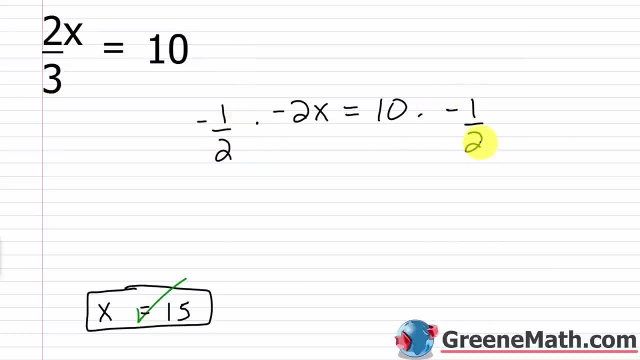 I can do that. But really, it's kind of just faster just to divide in this scenario, right? 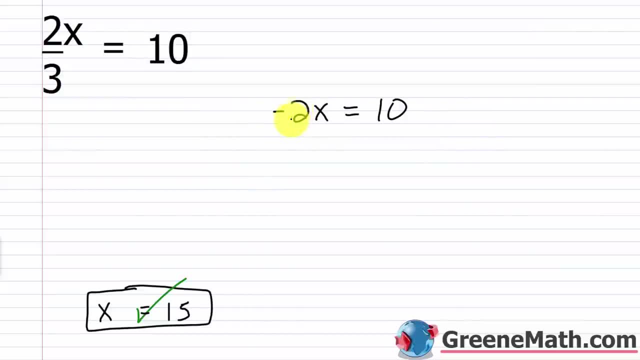 So in this scenario, I wouldn't do that. I would just say, OK, the coefficient of x is negative 2. So to get x by itself, I would divide both sides of the equation by negative 2. Because negative 2 divided by negative 2 is 1. So I'd have 1 times x, or just x. 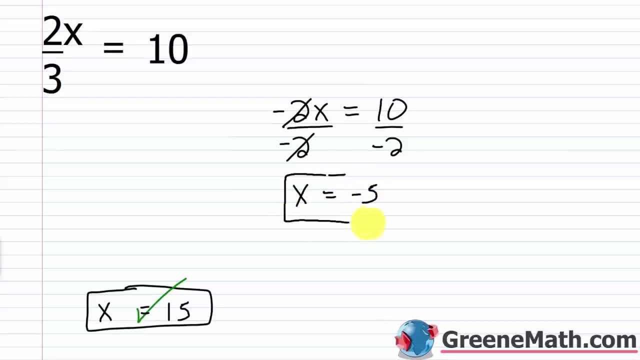 Then 10 divided by negative 2 is negative 5. So in this case, the solution would be x equals negative 5. 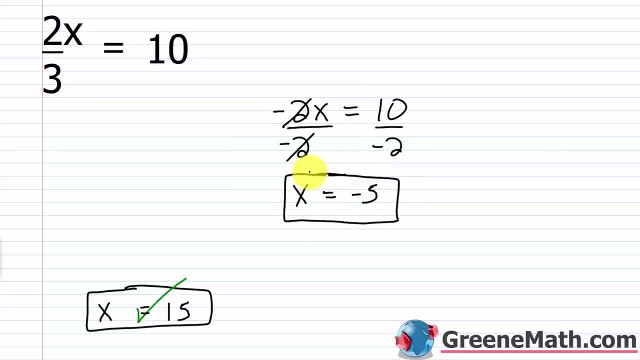 So again, if you have a fractional coefficient for your variable, you want to multiply both sides of the equation by the reciprocal of that fraction. 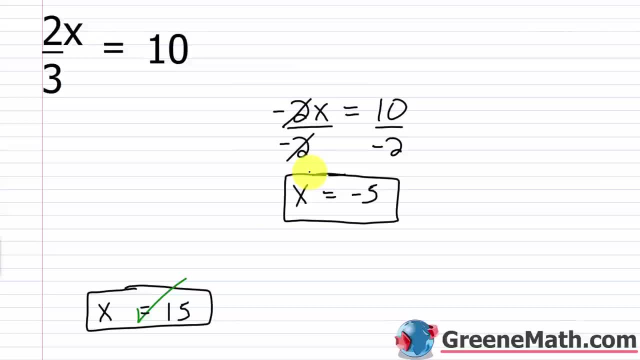 If you have an integer coefficient, you just want to divide both sides of the equation by that integer. OK. All right. Let's look at the next one. 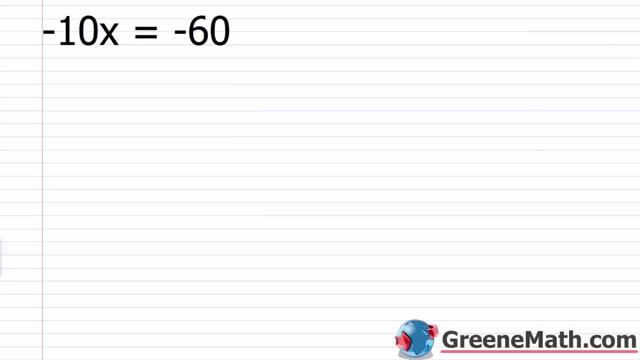 So we have negative 10x equals negative 60. So here's an example where we have an integer coefficient. We have negative 10. That's multiplying x. So to isolate my variable x, to isolate x, I would divide both sides of the equation by negative 10. 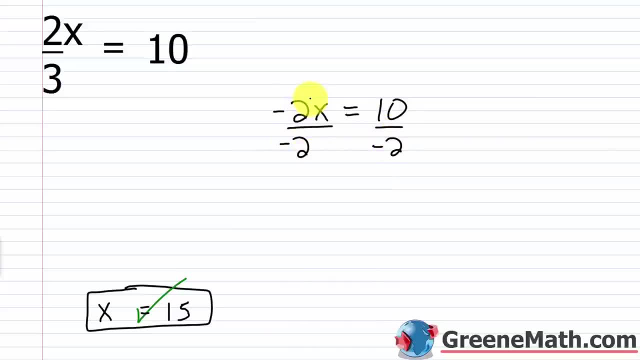 of the equation by negative 2. Because negative 2 divided by negative 2 is 1. So I'd have 1 times x or just x. Then 10 divided by negative 2 is negative 5. So in this case the solution would be: x equals negative 5.. 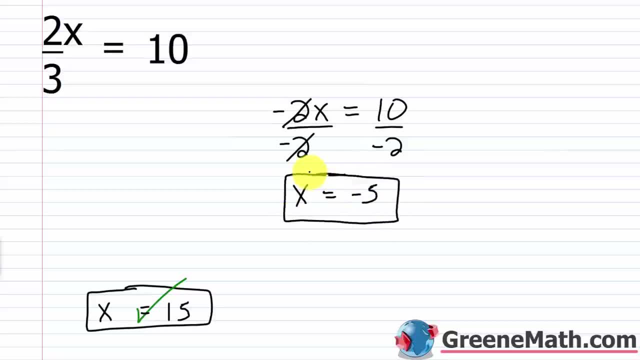 So again, if you have a fractional coefficient for your variable, you want to multiply both sides of the equation by the reciprocal of that fraction. If you have an integer coefficient, you just want to divide both sides of the equation by that integer. 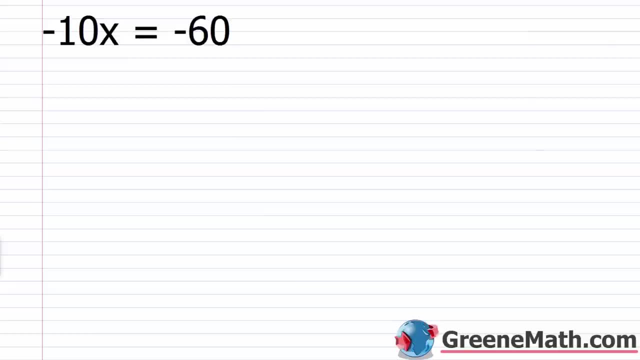 All right, let's look at the next one. So we have negative 10x equals negative 60.. So here's an example: where we have an integer coefficient right, We have negative 10.. That's multiplying x. So to isolate my variable x, to isolate x, 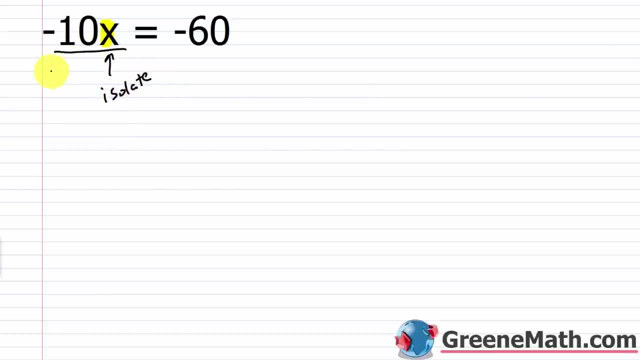 I would divide both sides of the equation by negative 10.. So if I divide this side by negative 10 and this side by negative 10, this will cancel with this and give me 1.. 1 times x is just x. 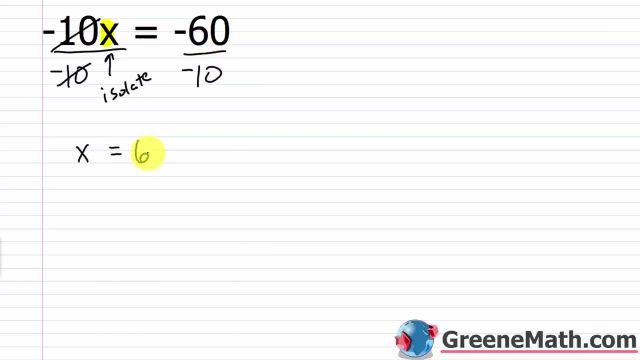 Over here. negative 60 divided by negative 10 is just 6.. And that's how quick I get my solution right. x equals 6. And if you check this, you just plug back in for x. plug a 6 in there. 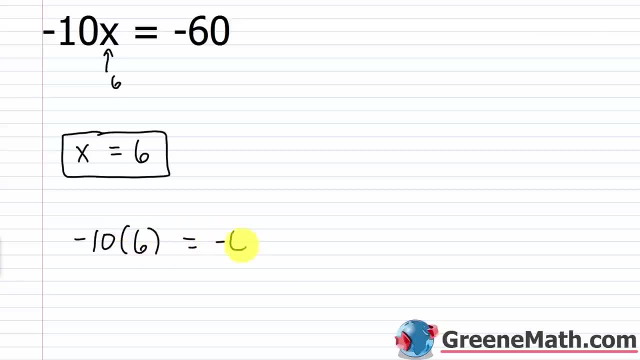 Well, I'd have: negative 10 times 6 equals negative 60. Of course that's true Negative times. positive is negative. 10 times 6 is 60. So I get negative 60 equals negative 60. And so we can say this solution here: x equals 6, is correct. 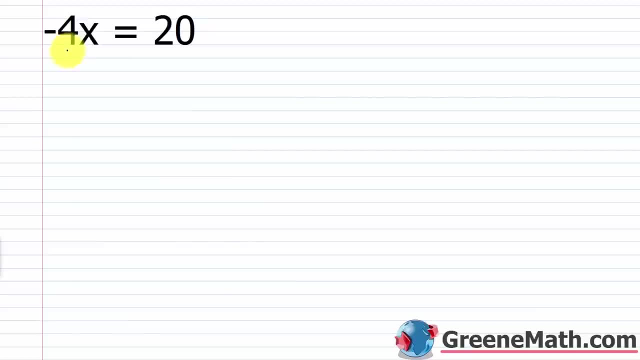 All right, what about negative? 4x equals 20? So again I have an integer coefficient for x. So if negative 4 is multiplying x, and I want x by itself, again I want to isolate. I want to isolate my variable x. 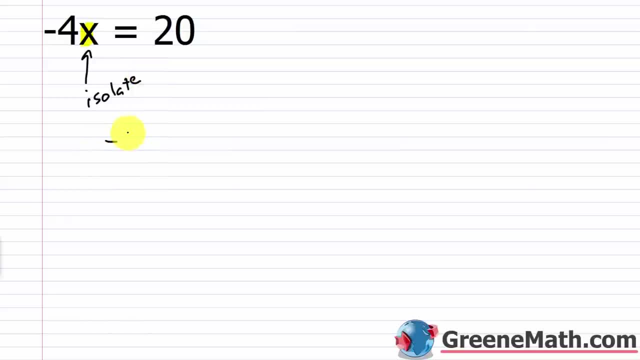 Well, I'm just going to divide both sides of the equation by negative 4, right, The coefficient of x. Really, that's simple, because negative 4 divided by negative 4 is going to give me 1, right. 1 times x is just x. 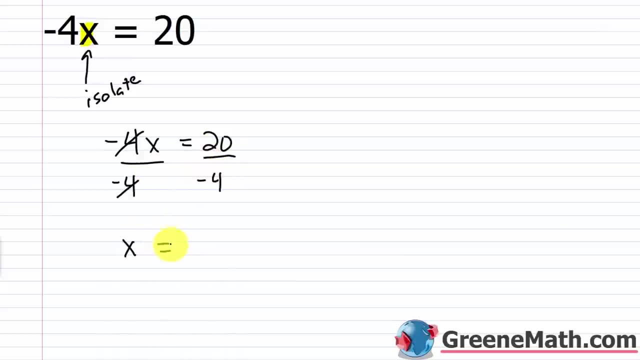 All right, And I've got to make sure I do it to this side. So then I have: x is equal to 20 divided by negative. 4 is negative 5.. Plug negative 5 back in for x in the original equation. 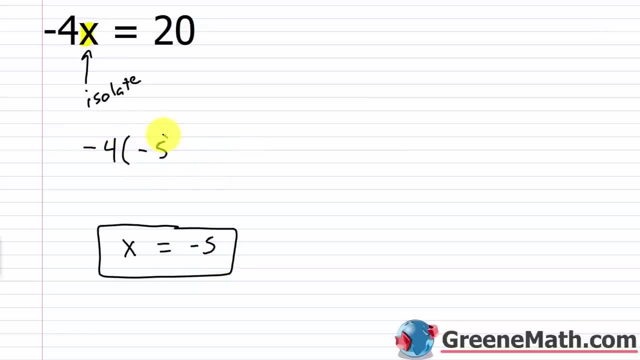 So you will have negative 4 times negative. 5 equals 20.. Negative times negative is positive. 4 times 5 is 20.. So 20 equals 20.. So, yeah, this is the correct solution: x equals negative, 5.. 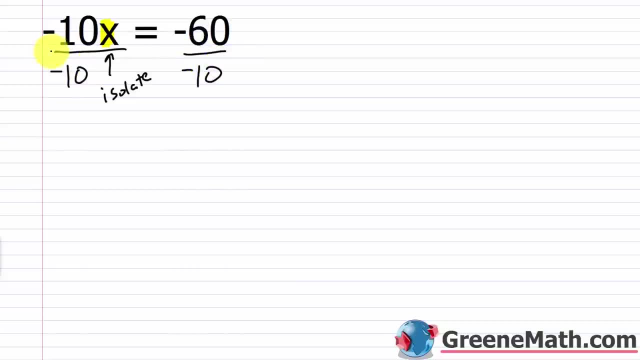 So if I divide this side by negative 10 and this side by negative 10, this will cancel with this and give me 1. 1 times x is just x. Over here. 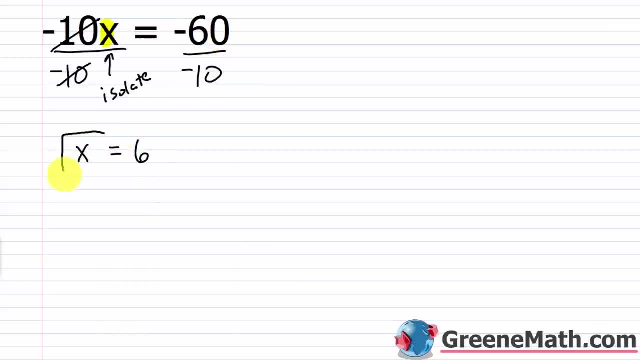 Negative 60 divided by negative 10 is just 6. And that's how quick I get my solution, right? 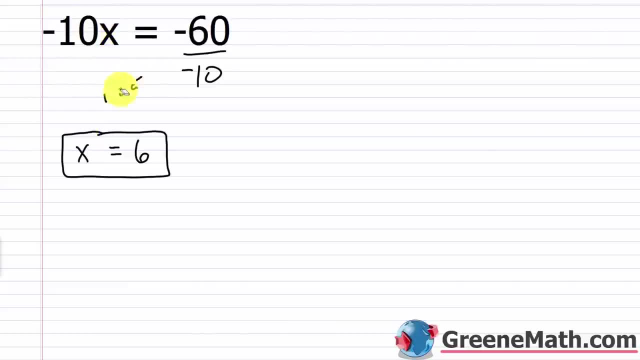 x equals 6. And if you check this, you just plug back in for x. 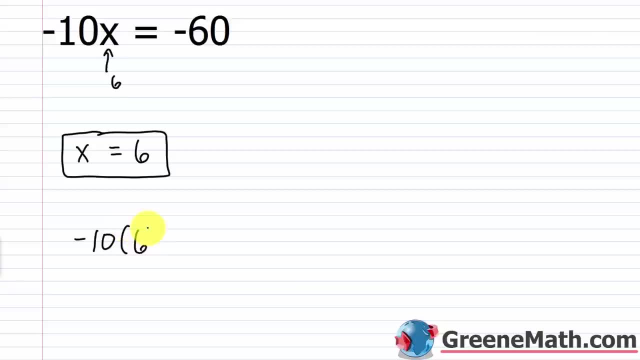 Plug a 6 in there. Well, I'd have negative 10 times 6 equals negative 60. Of course, that's true. Negative times positive is negative. 10 times 6 is 60. So I get negative 60 equals negative 60. And so we can say this solution here, x equals 6, is correct. All right. What about negative 4x equals 20? So again, we have negative 4x equals 20. 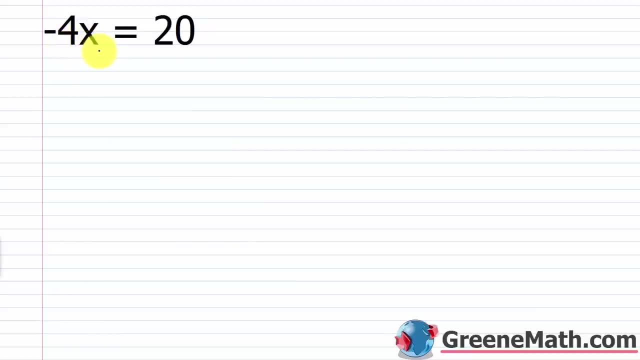 All right. So again, I have an integer coefficient for x. So if negative 4 is multiplying x, and I want x by itself, again, I want to isolate. I want to isolate my variable x. Well, I'm just going to divide both sides of the equation by negative 4, right? The coefficient of x. Really, that's simple because negative 4 divided by negative 4 is going to give me 1, right? 1 times x is just x. 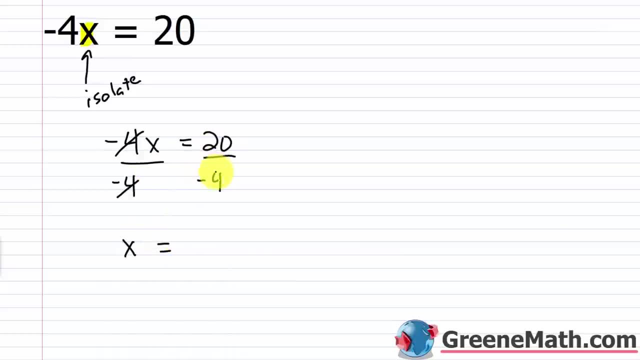 And I've got to make sure I do it. I'm going to go to this side, so then I have x is equal to 20 divided by negative 4 is negative 5. Plug negative 5 back in for x in the original equation. So you will have negative 4 times negative 5 equals 20. Negative times negative is positive. 4 times 5 is 20. So 20 equals 20. So yeah, this is the correct solution. x equals negative 5. All right. 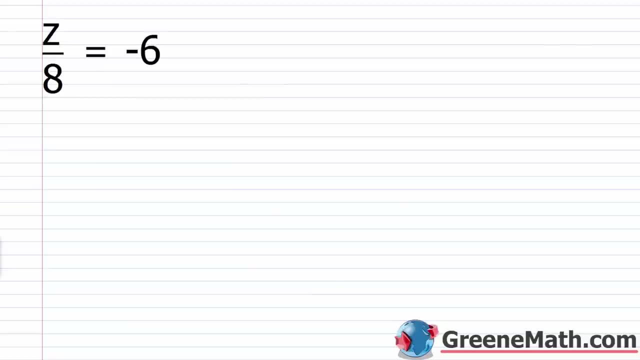 What about something like z over 8 equals negative 6? So the first thing is you've got to realize, if I have z over 8, I can think of a way to do this. I can think of a way to do this. I can think about it as z divided by 8. Or I can really think about this as 1 eighth times z equals negative 6. So if I think about it as 1 eighth times z, well, yeah, this is a fractional coefficient for z. 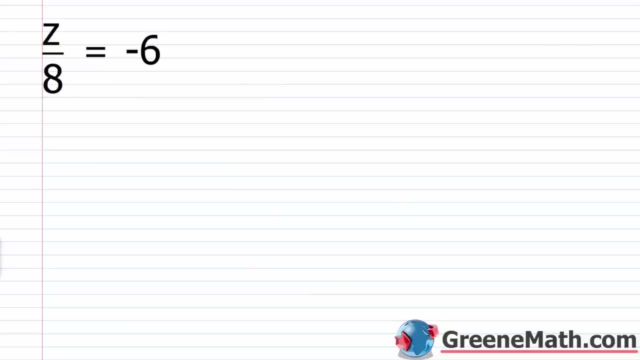 All right. what about something like z over 8 equals negative 6?? So the first thing is, you've got to realize, if I have z over 8, I can think about it as z divided by 8, or I can really think about this as 1 eighth times z equals negative 6.. 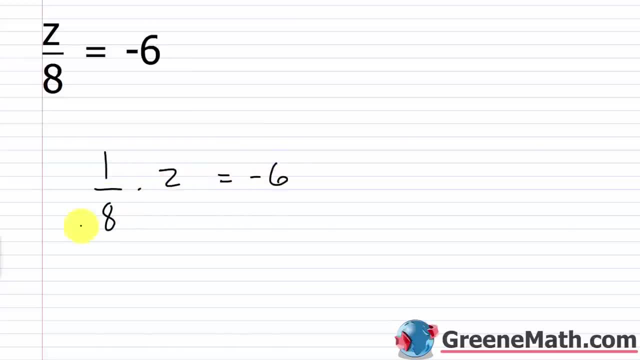 So if I think about it as 1 eighth times z, well, yeah, this is a fractional coefficient for z. Remember, we talked about the fact that if you had a fractional coefficient for your variable, when you go to think about isolating the variable, 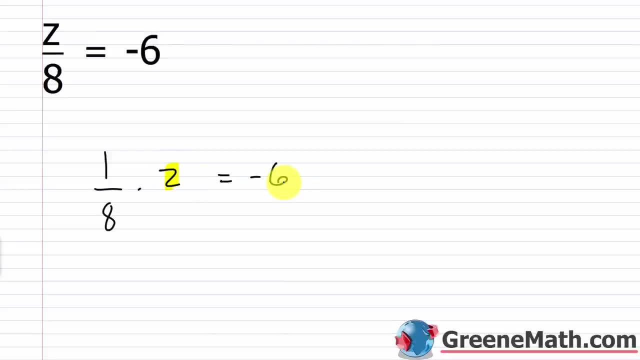 I would just multiply both sides by the reciprocal of that fractional coefficient. So the reciprocal of 1 eighth is 8 over 1, or just 8.. So times 8 over 1, times 8 over 1.. So this will cancel and you'll just have z on the left side. 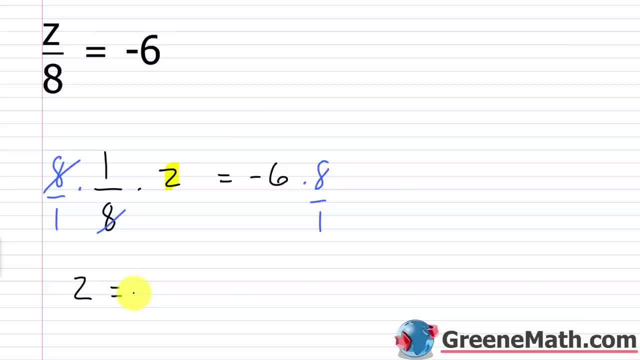 On the right. negative 6 times 8 over 1 is the same as negative 6 times 8. That's negative 48.. Now another way to kind of think about this, and again, there's multiple ways to look at it. 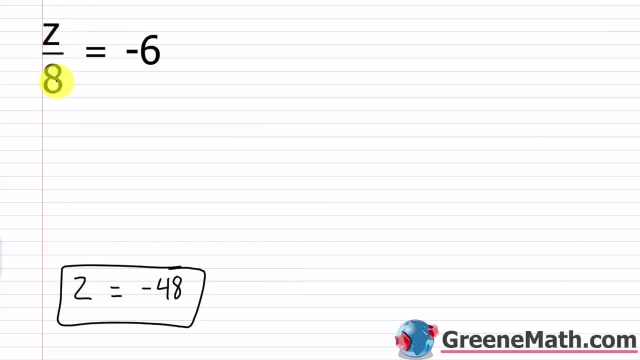 I have z divided by 8. So kind of to get z by itself. since it's divided by 8, I need to multiply by 8, kind of to undo the division. So you can think about it as multiplication undoing division. 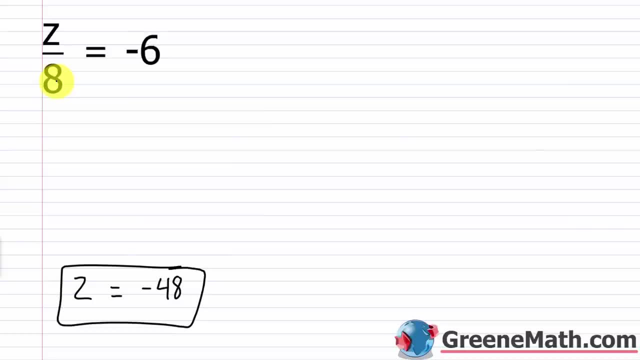 division undoing multiplication. right, You always want to do kind of the opposite operation. So since I have z and I'm dividing by 8, to undo that I multiply by 8. And because I do it to this side, I must also do it to this side. 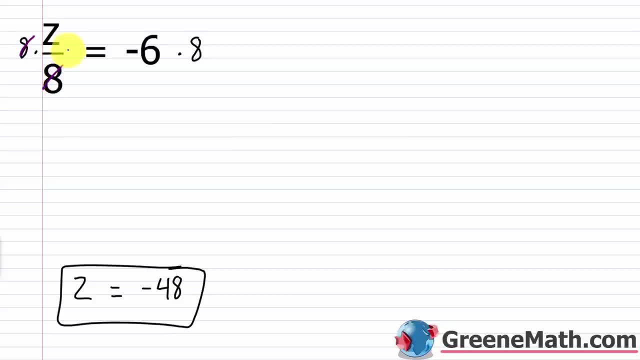 So then this will cancel with this right: 8 over 8 is just 1.. 1 times z is just z, And negative 6 times 8, again is negative 48.. So kind of, either way you think about that. 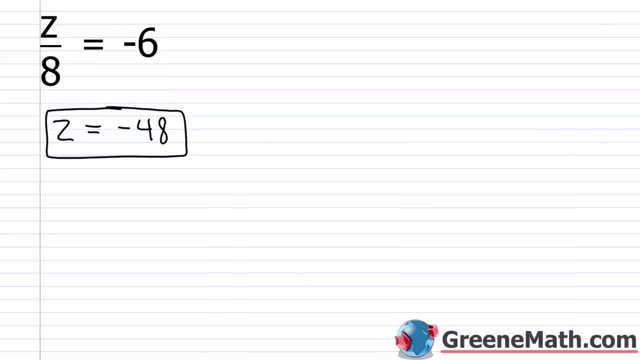 you get z equals negative 48 as your solution. All right, so let's check our solution of z equals negative 48.. So again, I'm just going to take negative 48, and I'm going to plug it in for z. 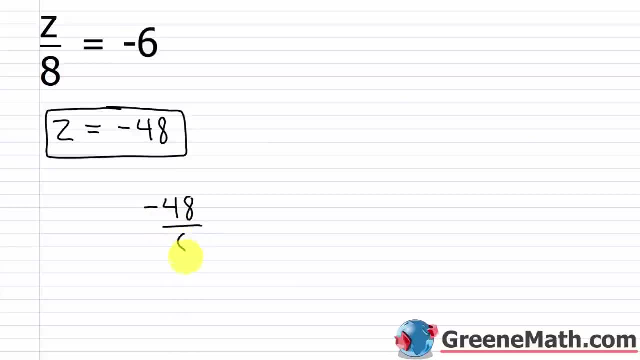 So I would have: negative 48 divided by 8 equals negative 6.. And of course, we can already see that this is true. A negative divided by a positive is a negative. 48 divided by 8 is 6.. So I'd have: negative 6 is equal to negative 6.. 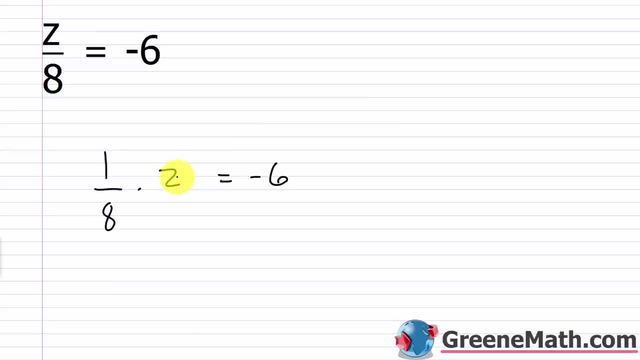 Remember, we talked about the fact that if you had a fractional coefficient for your variable, when you go to think about isolating the variable, I would just multiply both sides by the reciprocal of that fractional coefficient. 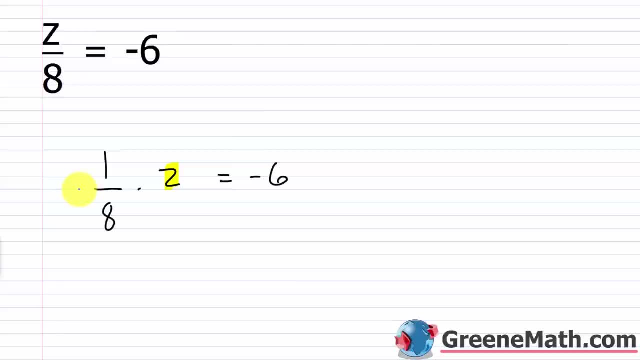 So the reciprocal of 1 eighth is 8 over 1, or just 8. 8 times 8 over 1 times 8 over 1. So this will cancel, and you'll just have z on the left side. 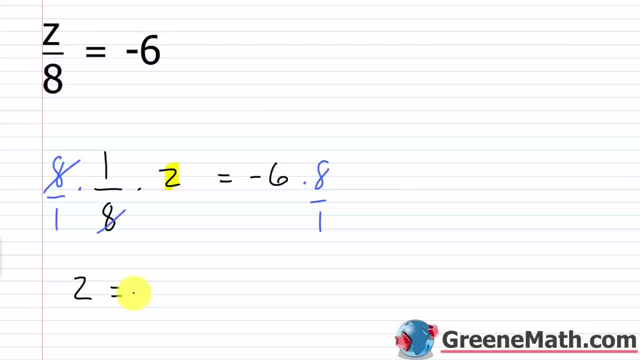 On the right, negative 6 times 8 over 1 is the same as negative 6 times 8. 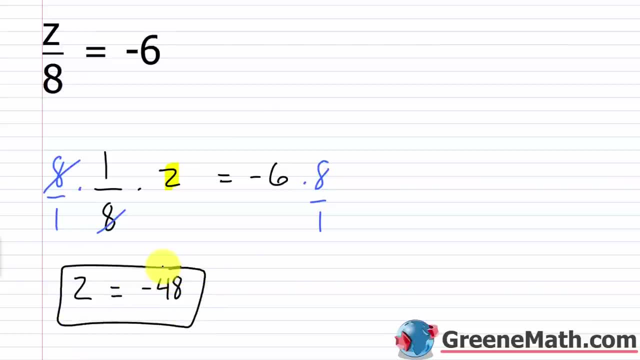 That's negative 48. Now another way to kind of think about this, and again, there's multiple ways to look at it. 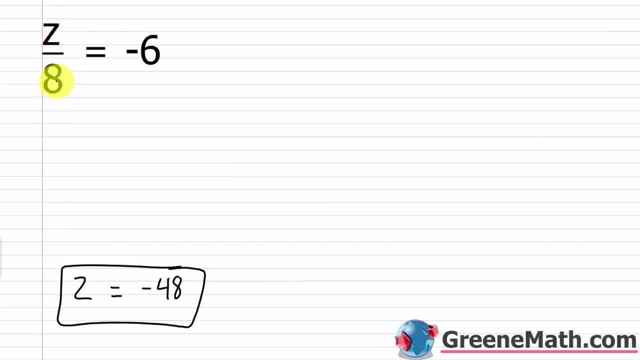 I have z divided by 8. So kind of to get z by itself, since it's divided by 8, I need to multiply by 8. Kind of to undo the division. So you can think about it as multiplication undoing division, division undoing multiplication. You always want to do kind of the opposite operation. So since I have z and I'm dividing by 8, to undo that, I multiply by 8. And because I do it to this side, I must also do it to this side. So then this will cancel with this. 8 over 8 is just 1. 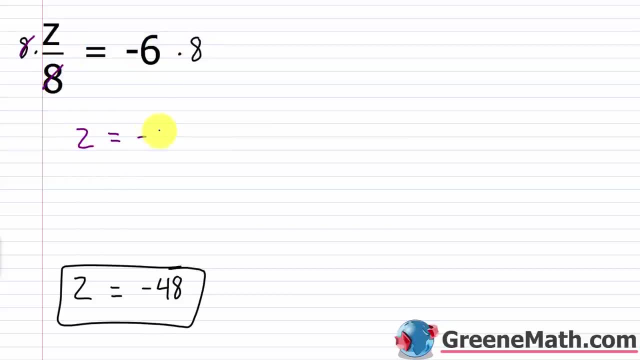 1 times z is just z. And negative 6 times 8, again, is negative 48. 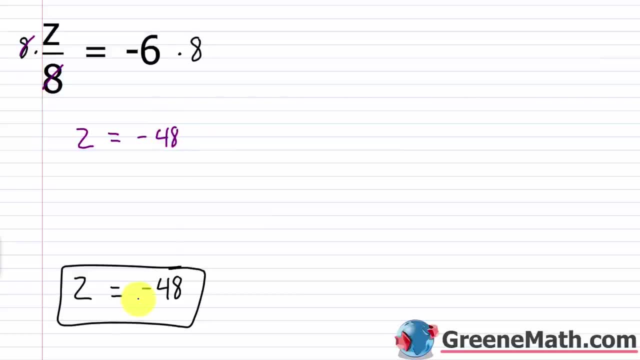 So kind of either way you think about that. You get z equals negative 48 as your solution. 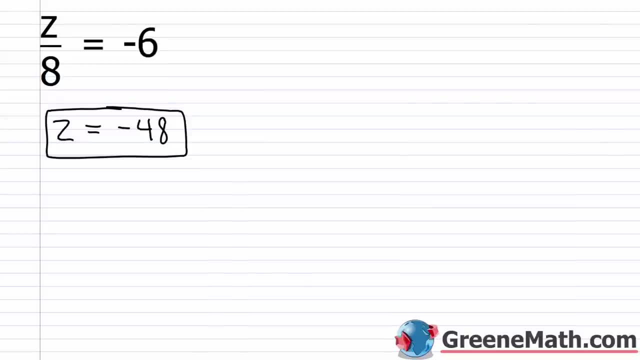 All right, so let's check our solution of z equals negative 48. So again, I'm just going to take negative 48 and I'm going to plug it in for z. So I would have negative 48 divided by 8 equals negative 6. And of course, we can already see that this is true. A negative divided by a positive is a negative. 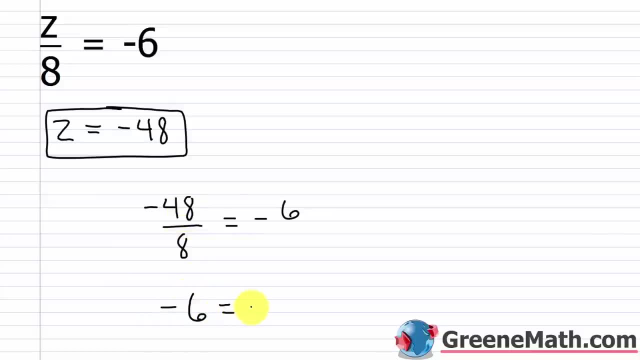 48 divided by 8 is 6. So I'd have negative 6 is equal to negative 6. 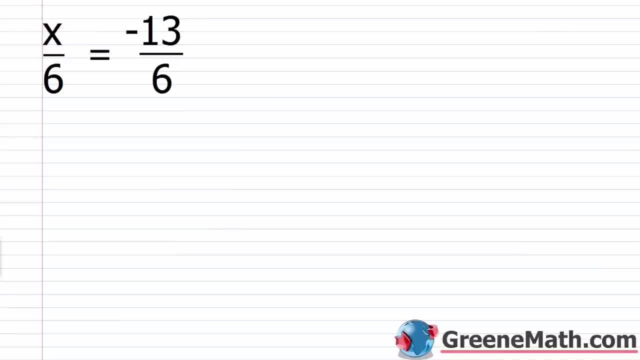 All right, let's take a look at one final problem. So we have x over 6 is equal to negative 13 over 6. 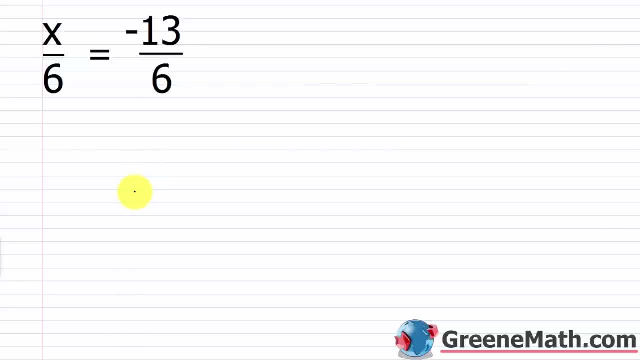 So again, I can think about this in multiple ways. I can just say, OK, I have x divided by 6. So to undo the division, I can use multiplication. So x over 6 equals negative 13 over 6. Since I'm dividing x by 6, I can multiply by 6. 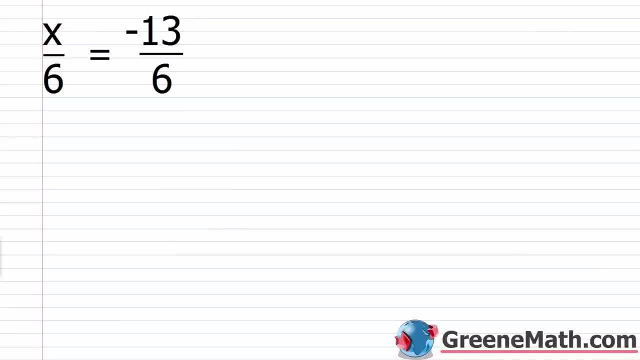 All right, let's take a look at one final problem. So we have: x over 6 is equal to negative 13 over 6.. So again, I can think about this in multiple ways. I can just say: okay, I have x divided by 6.. 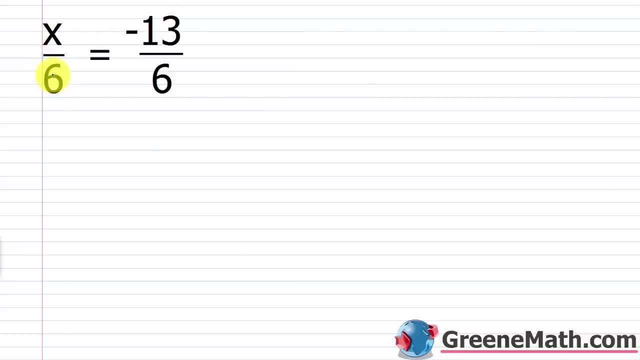 So to undo the division I can use multiplication. So x over 6 equals negative 13 over 6.. Since I'm dividing x by 6, I can multiply by 6, right, 6 over 6 would be 1, right. 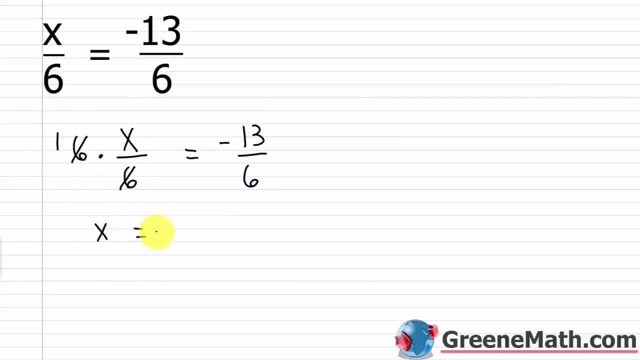 Those would cancel And I'd have 1 times x or just x on the left. But again, to make this legal I've got to also multiply by 6 on the right side And then 6 would cancel with 6 here and give me 1.. 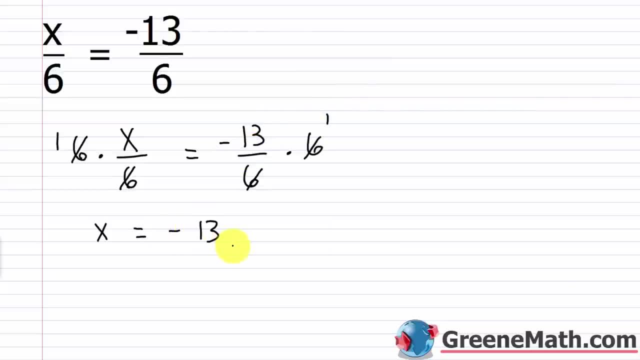 1 times negative, 13 is negative 13.. So x equals negative, 13 is the solution. Now, another way you could have thought about this: if I see a variable over a number, remember- I can break that up and say: 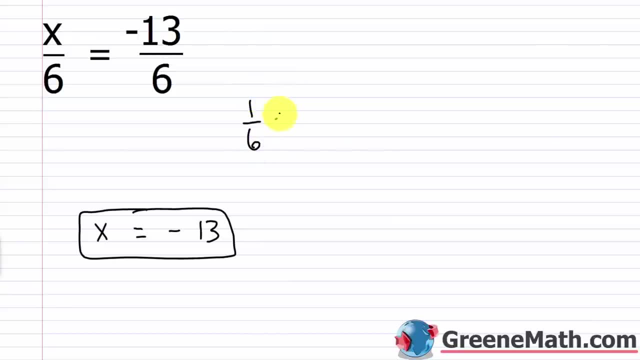 okay, well, this is the same as if I had 1 sixth times x equals negative 13 over 6.. For some students, that'll make it mentally easier for you to say: okay, well, I have this times this, So I know that I can multiply both sides by the reciprocal if I have a fractional coefficient for x. 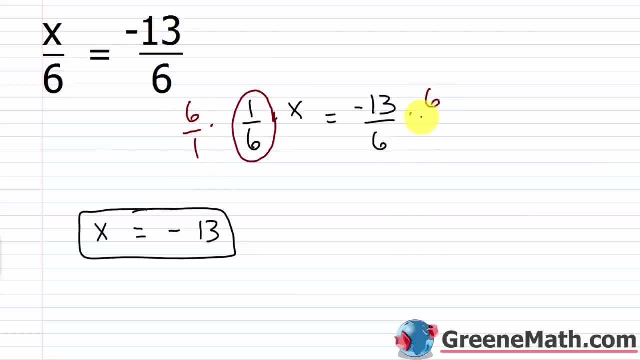 So I can multiply both sides by 6 over 1.. And multiplying by 6 over 1 is the same thing as what we did earlier when we multiplied by 6, right, It's the same thing, It's just. this might be mentally easier for you to remember. 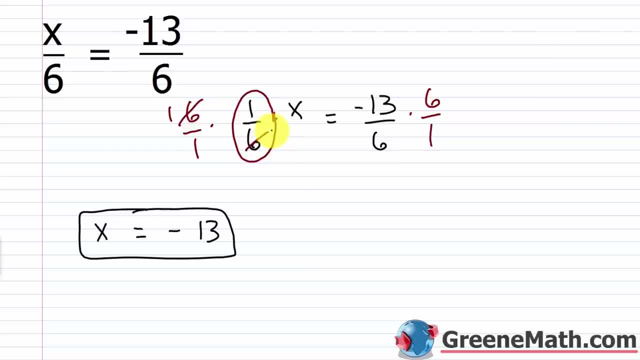 So then this will cancel with this and give me a 1.. So 1 times x is just negative 13.. x is just x. And then over here, this will cancel with this and give me 1. 1 times negative 13 is negative 13.. 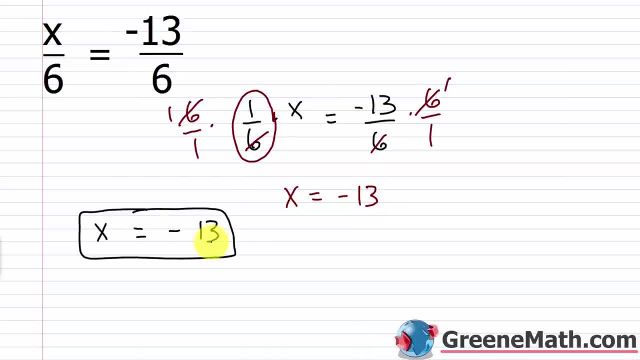 So again, either way you do it, you're going to get that x equals negative 13. And when we check this problem, if I plug a negative 13 up here- well look how easy it is to see- I would have negative 13 over 6, right. 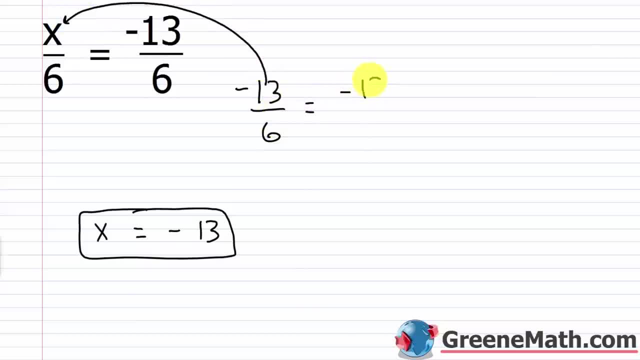 Again. I just plug this in, for x equals negative 13 over 6.. Yeah, same value on the left and the right. So our solution here, x equals negative 13,, is of course correct. Hello and welcome to Algebra 1,, Lesson 5.. 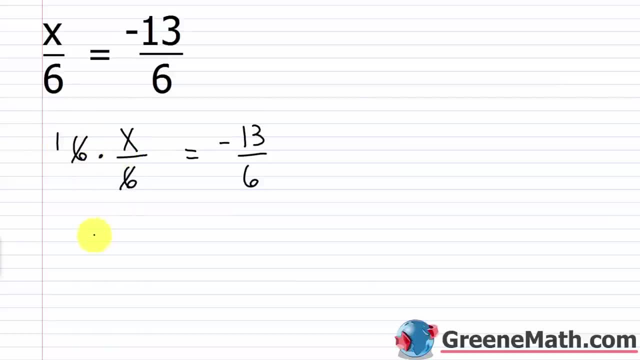 6 over 6 would be 1. Those would cancel. And I'd have 1 times x, or just x on the left. But again, to make this legal, I've got to also multiply by 6 on the right side. And then 6 would cancel with 6 here and give me 1. 1 times negative 13 is negative 13. So x equals negative 13 is the solution. 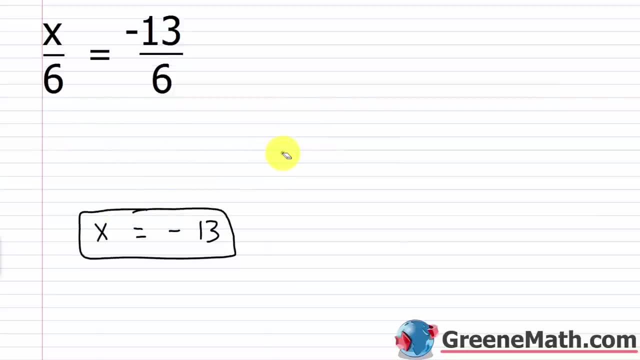 Now another way you could have thought about this, if I see a variable over a number, remember, I can break that up and say, OK, well, this is the same as if I had 1 sixth times x equals negative 13 over 6. For some students, that'll make it mental. 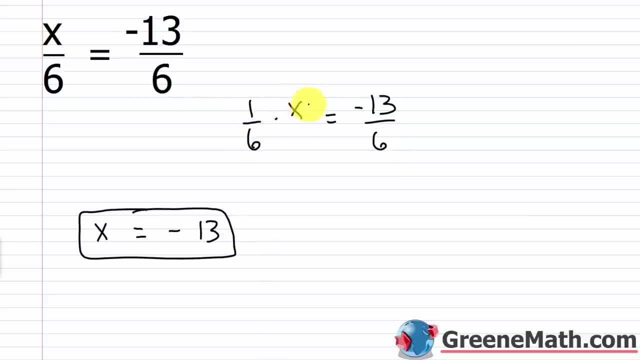 It'll make it mentally easier for you to say, OK, well, I have this times this. So I know that I can multiply both sides by the reciprocal if I have a fractional coefficient for x. So I can multiply both sides by 6 over 1. And multiplying by 6 over 1 is the same thing as what we did earlier when we multiplied by 6. It's the same thing. 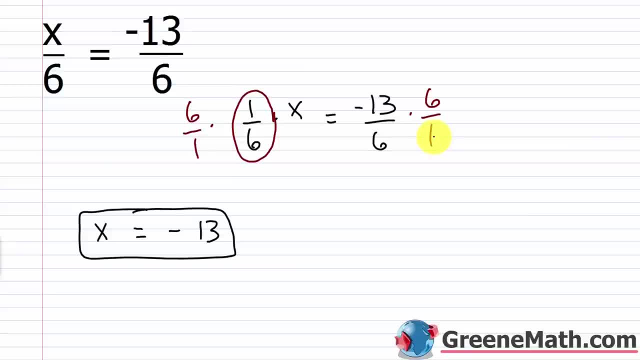 It's just this might be mentally easier for you to remember. 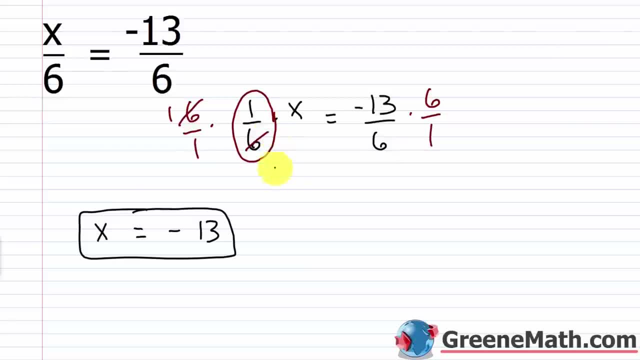 So then this will cancel with this and give me a 1. So 1 times x is just x. And then over here. It'll cancel with this and give me 1. 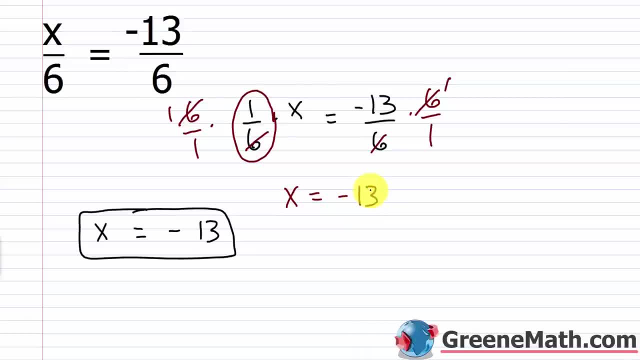 1 times negative 13 is negative 13. So again, either way you do it, you're going to get that x equals negative 13. 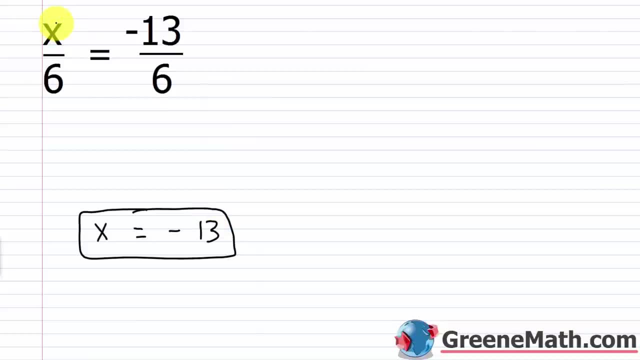 And when we check this problem, if I plug a negative 13 up here, well, look how easy it is to see. I would have negative 13 over 6. 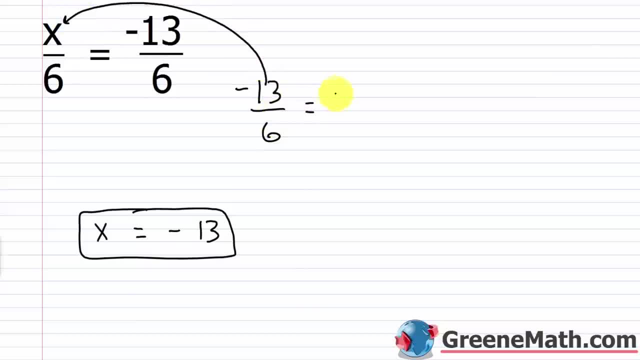 All right, again, I just plug this in for x equals negative 13 over 6. Yeah, same value on the left and the right. So our solution here, x equals negative 13, is, of course, correct. 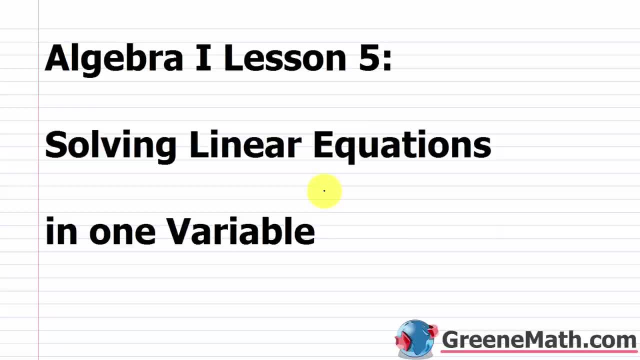 Hello. And welcome to Alcestor. Algebra 1, Lesson 5. In this video, we're going to learn about solving linear equations in one variable. 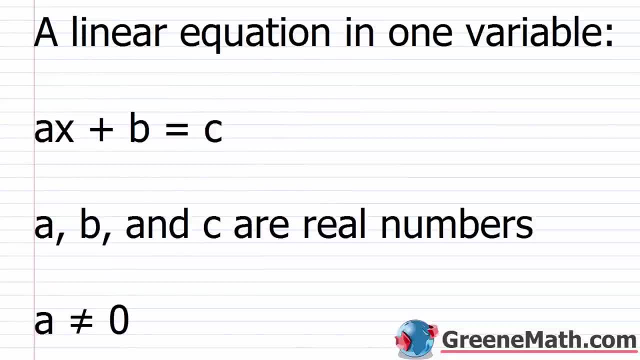 OK, so in the last two lessons, we've learned how to solve very simple versions of a linear equation in one variable. 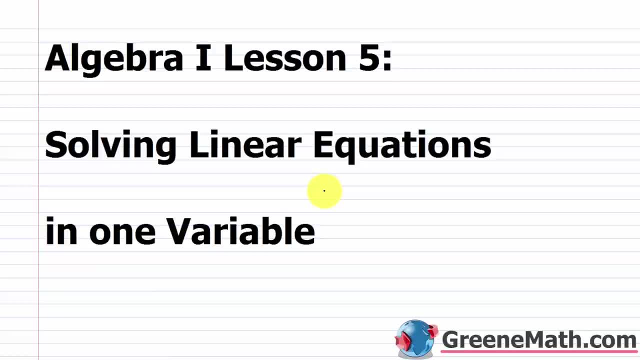 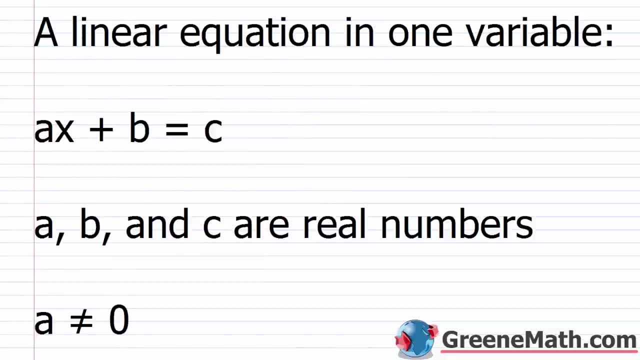 In this video we're going to learn about solving linear equations in one variable. Okay, so in the last two lessons we've learned how to solve very simple versions of a linear equation in one variable. So we kind of started out by learning something known as the addition property of equality. 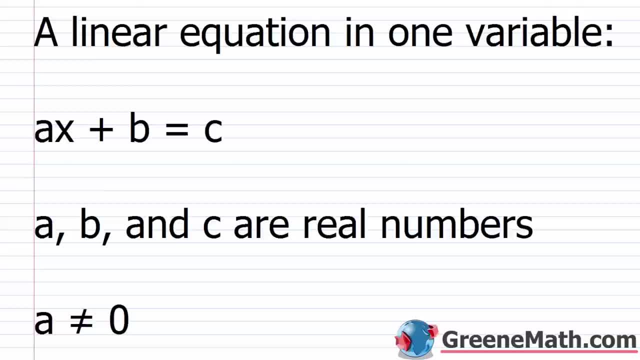 And then we moved on to talk about the multiplication property of equality. But in this lesson we're going to combine the two And learn how to solve any linear equation in one variable. So let me first define what a linear equation in one variable is. 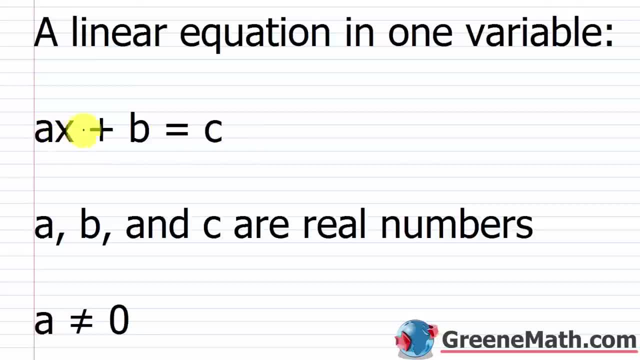 It looks like this, And you're probably going to see this in your textbook: ax plus b equals c. Now, in the previous two lessons, you probably heard me say that a, b and c are real numbers, And we really haven't talked about what a real number is yet. 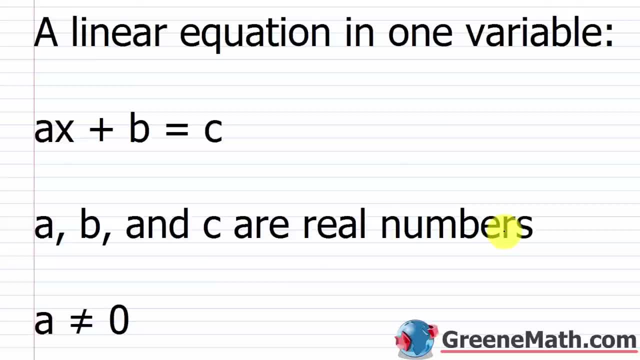 But for right now, just think of it as any number that you can think of. So now let's kind of move on. Okay, move further in this definition, and we're going to put a restriction on a. So that's this right. 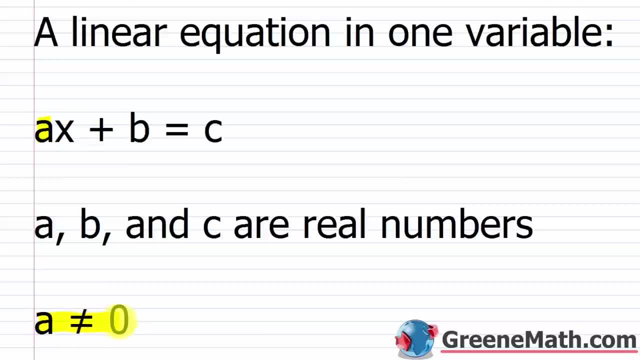 here. So you see here, where I have, a does not equal zero. And why can't a be zero? Well, if I plug a zero in for a, I would have zero times x, and zero times x is zero. So then I just have b. 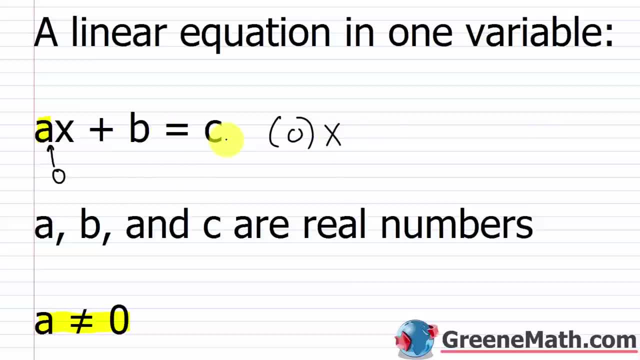 equals c, And that's not going to work unless b and c are the same number, And in almost every case they're not going to be. So again, let me reiterate: ax plus b equals c is kind of our general form for a linear equation in one variable where a, b and c are real numbers. So 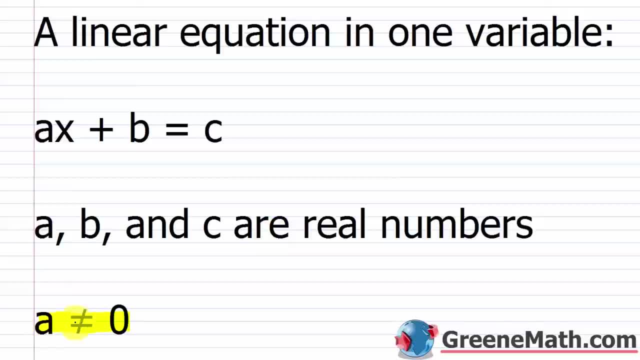 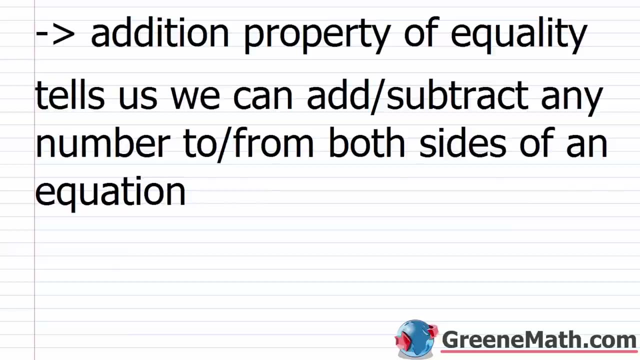 any numbers that you can think about, and a can never be zero. So this can never, never be zero. All right, let's talk a little bit about the addition property of equality. Again, this tells us that we can add or subtract any number to or, in the case of subtraction from, 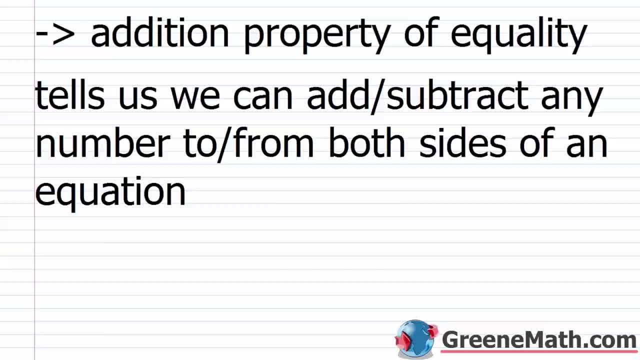 both sides of an equation And remember we use it to solve these simple equations that look like this: x plus 4 equals 7, right? So in this case, we have 4 that's being added to x. We want to. 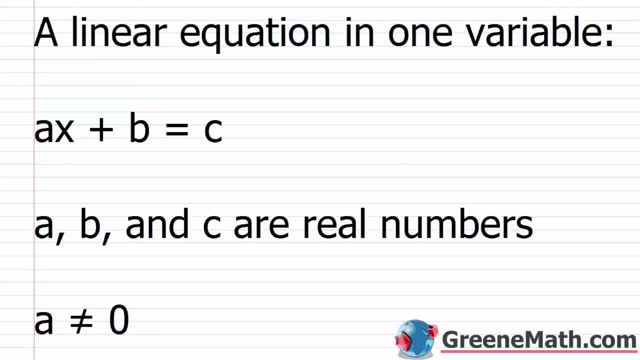 So we kind of started out by learning something known as the addition property of equality. And then we moved on to talk about the multiplication property of equality. 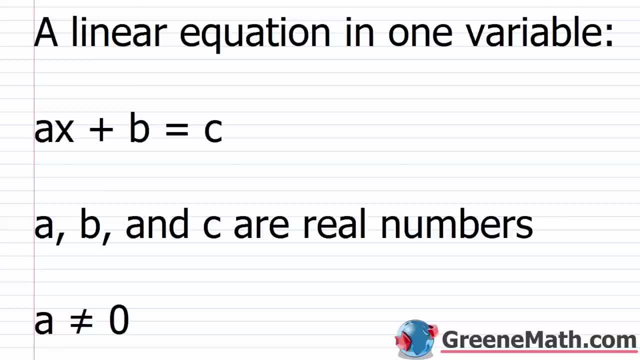 But in this lesson, we're going to combine the two and learn how to solve any linear equation in one variable. So let me first define what a linear equation in one variable is. It looks like this. And you're probably going to see this in your textbook. Ax plus b equals c. Now in the previous two lessons, you probably heard me say that a, b, and c are real numbers. 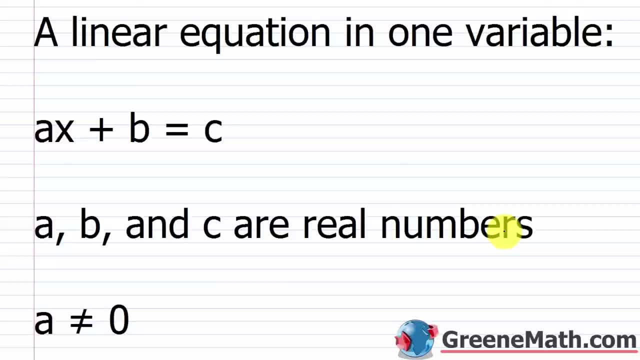 And we really haven't talked about what a real number is yet. But for right now, just think of it as any number that you can think of. So now let's kind of move further in this definition. And we're going to plug this in. OK. 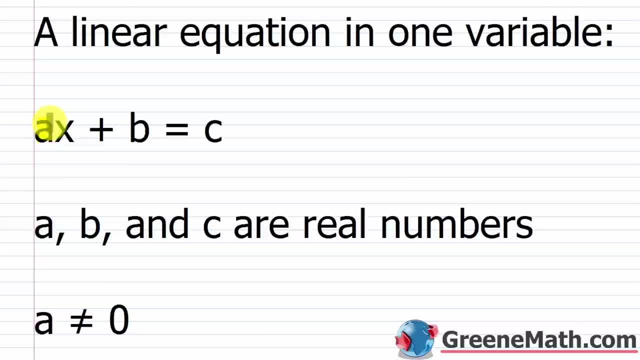 Let's put a restriction on a. So that's this right here. So you see here where I have a does not equal 0. And why can't a be 0? Well, if I plug a 0 in for a, I would have 0 times x. 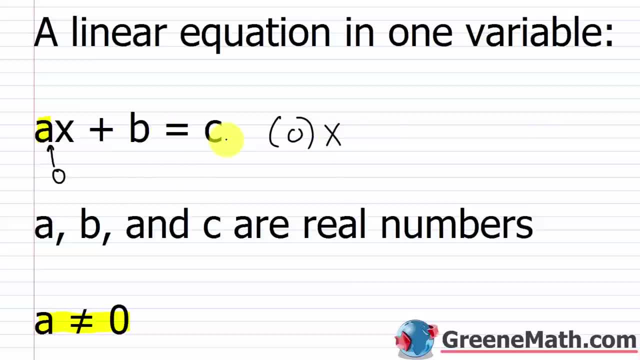 And 0 times x is 0. So then I just have b equals c. And that's not going to work unless b and c are the same number. 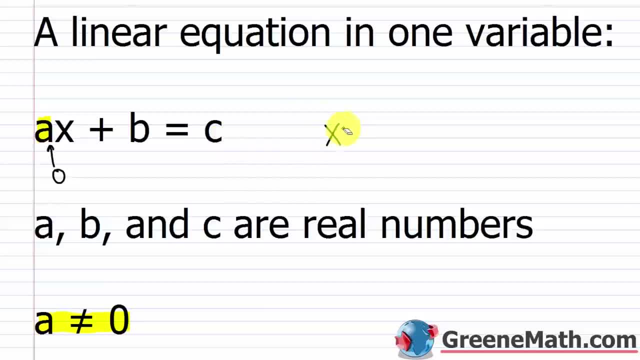 And in almost every case, they're not going to be. So again, let me reiterate. 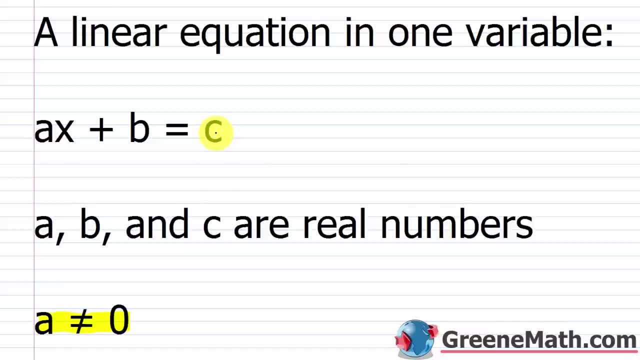 a, x plus b equals c is kind of our general form for a linear equation in one variable, where a, b, and c are real numbers. So any numbers that you can think about. And a can never be 0. 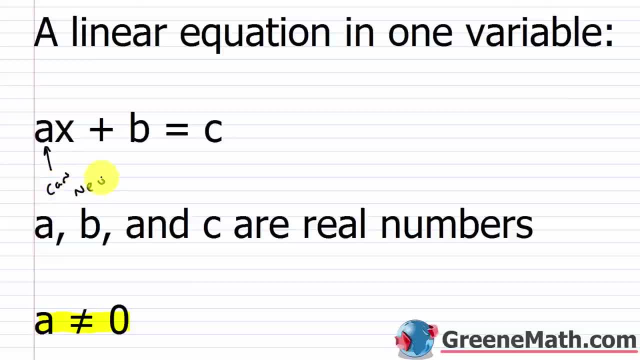 So this can never, never be 0. All right. 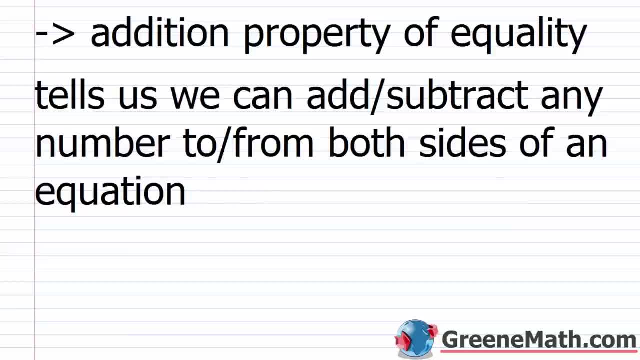 Let's talk a little bit about the addition property of equality. Again, this tells us that we can add or subtract any number to, or in the case of subtracting, subtraction from both sides of an equation. And remember, we use it to solve these simple equations that look like this. x plus 4 equals 7. So in this case, we have 4 that's being added to x. We want to isolate x. 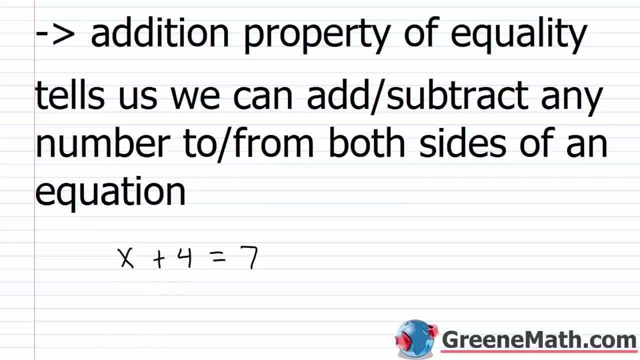 isolate x. So what we do is we subtract 4 from both sides of the equation. right, That's how we isolate x, Because we're adding 4 to x, we subtract 4, so x can be by itself, right 4 plus negative 4,. 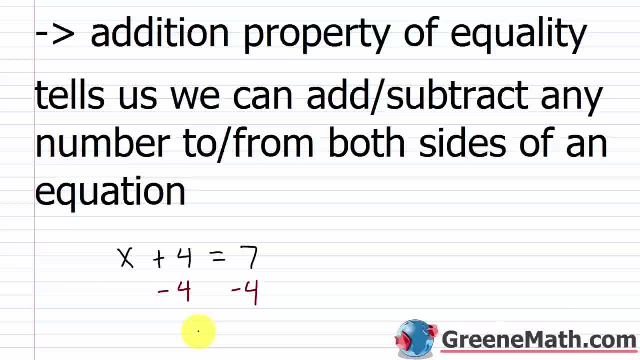 or 4 minus 4 is 0, and x plus 0 is just x. So I cancel this out here. This becomes a 0.. And then over here, 7 minus 4 is 3.. So let me scroll down a little bit and we have x equals 3.. 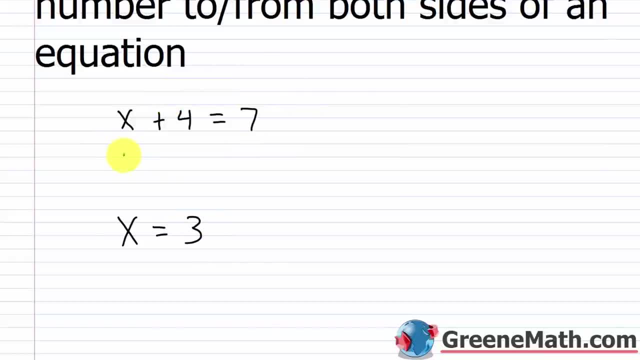 And I taught you how to check things. We plug the 3 in for x in the original equation: You'd have 3 plus 4, which is 7.. And then you plug the 3 in for x in the original equation, You'd have 3 plus 4,. 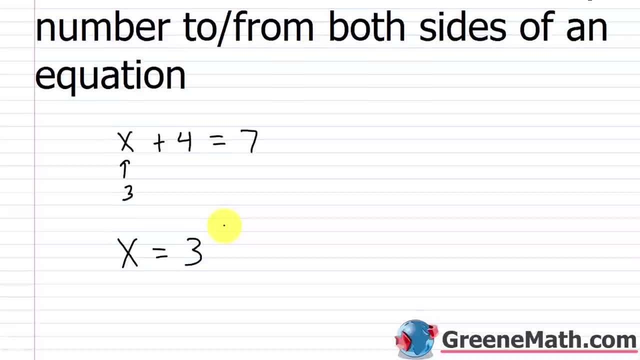 which is 7.. And then you plug the 3 in for x in the original equation You'd have 3 plus 4, which is 7. You'd have 7 equals 7.. So that checks out All right. so the other property that we've 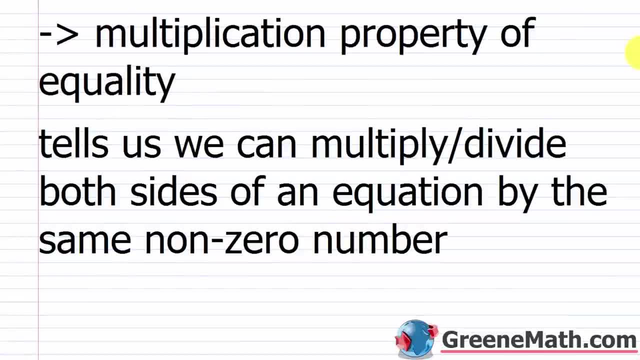 already talked about is the multiplication property of equality. Now this tells us that we can multiply or divide both sides of an equation by the same non-zero number. So you can't do it with 0, but anything else. So that's another example of a restriction. 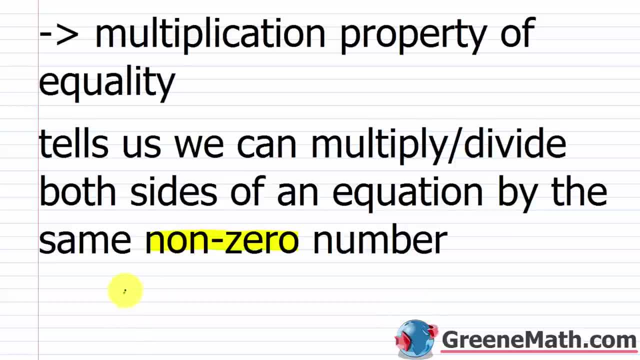 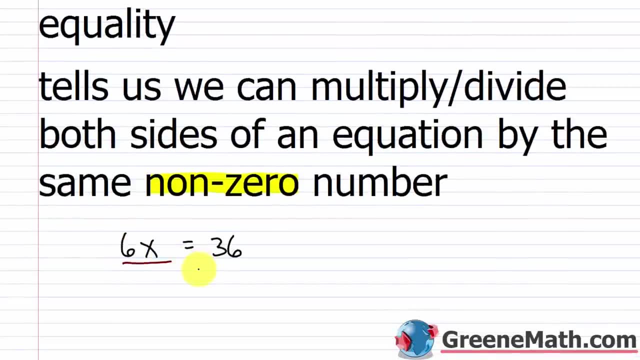 So we use this to solve stuff like 6x equals 36, right? So in this case I'm multiplying x by 6. So to kind of undo that and to get x by itself, I'm going to divide. All right, just think about the opposite operation, If I'm adding something to x. 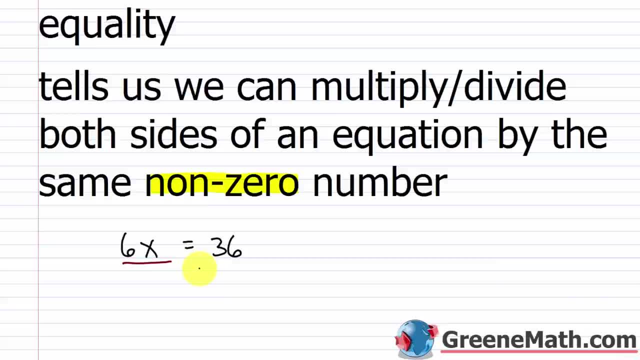 I want to subtract. If I'm subtracting away from x, I want to add. If I'm multiplying something by x, I want to divide. If I'm dividing x by something, I want to multiply. So in this case, I am multiplying x by 6.. So I want to divide by 6, right, I have to do that to both. 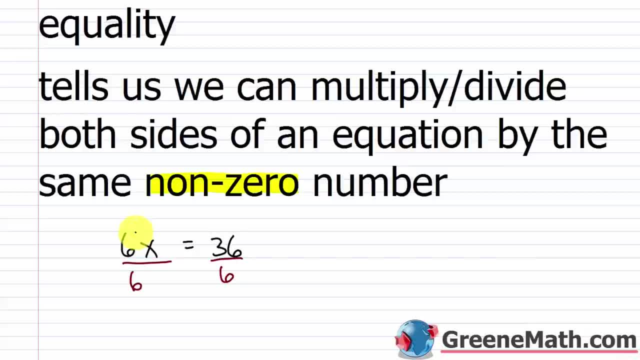 sides of the equation to preserve the solution. So this cancels with this and becomes 1.. 1x is just x. 36 divided by 6 is 6.. And of course, if you want to check this, if I plug the 6 in for x there, 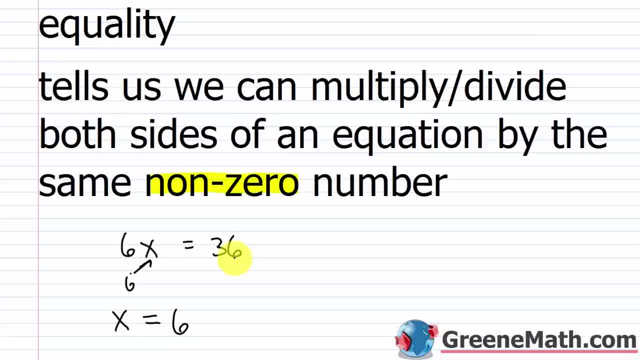 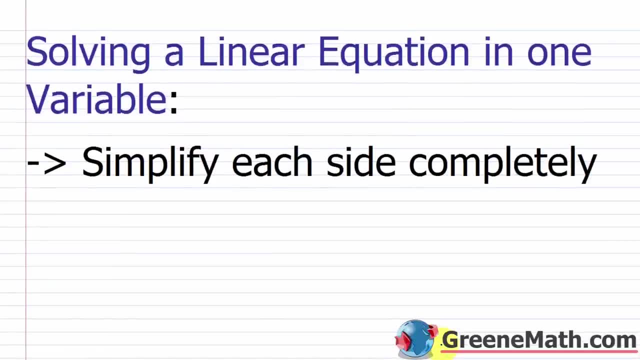 6 times 6 is 36.. You'd have 36 equals 36.. So that is correct, Okay, so now that we kind of have the hang of the basics, let's talk about a general procedure for solving a linear equation in one variable, And this is for any. 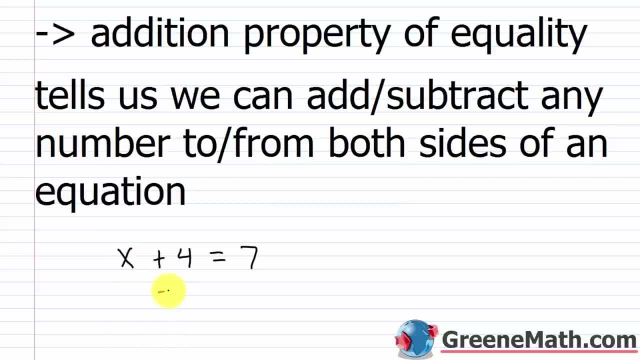 So what we do is we subtract. We subtract 4 from both sides of the equation. That's how we isolate x. Because we're adding 4 to x, we subtract 4. So x can be by itself. Right? x plus negative 4, or 4 minus 4 is 0. And x plus 0 is just x. So I cancel this out here. 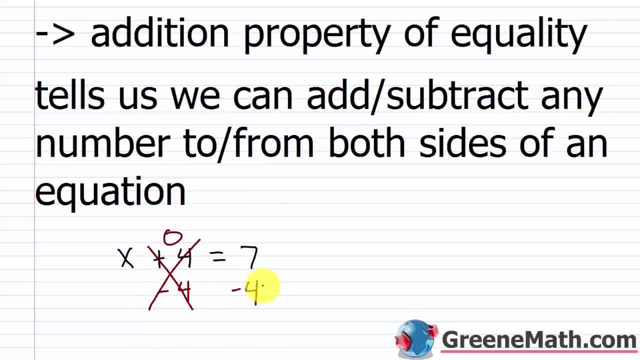 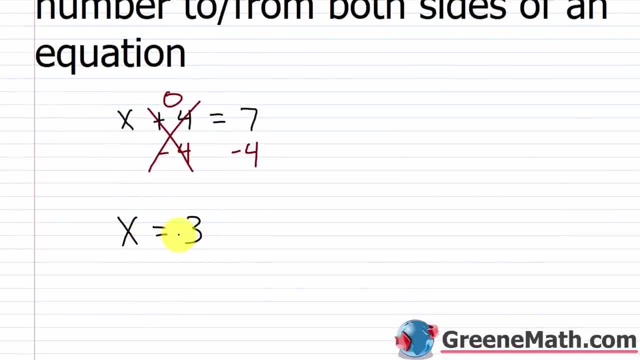 This becomes a 0. And then over here, 7 minus 4 is 3. So let me scroll down a little bit. And we have x equals 3. And I taught you how to check things. We plug the 3 in for x in the original equation. You'd have 3 plus 4, which is 7. You'd have 7 equals 7. So that checks out. All right. 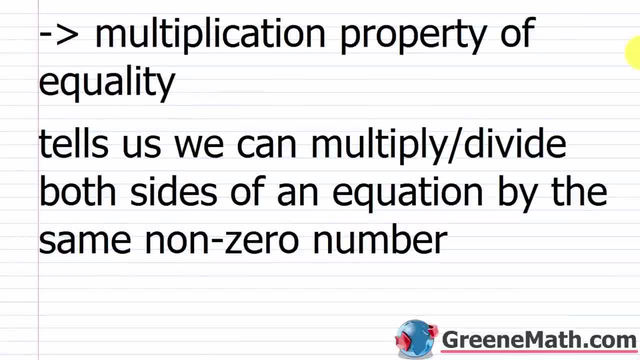 So what we're going to do now is we're going to do the multiplication property of equality. This tells us that we can multiply or divide both sides of an equation by the same non-zero number. So you can't do it with 0, but anything else. So that's another example of a restriction. So we use this to solve stuff like 6x equals 36. So in this case, I'm multiplying x by 6. So to undo that and to get x by itself, we're going to do the multiplication property of equality. So I'm going to divide x by itself. I'm going to divide. 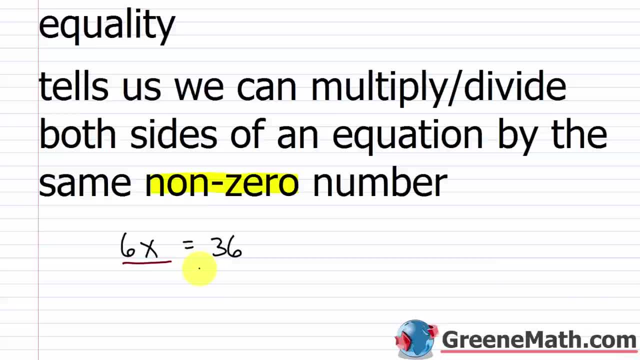 Just think about the opposite operation. If I'm adding something to x, I want to subtract. If I'm subtracting away from x, I want to add. If I'm multiplying something by x, I want to divide. If I'm dividing x by something, I want to multiply. So in this case, I am multiplying x by 6. So I want to divide by 6. 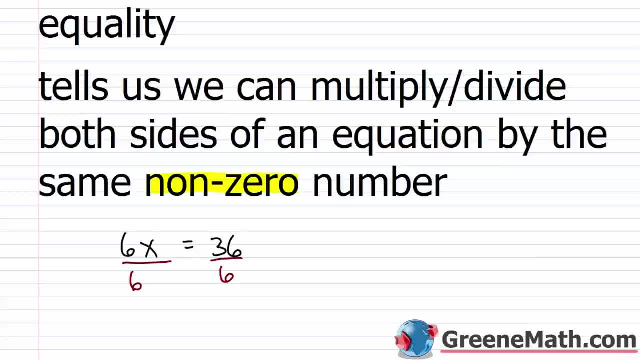 I have to do that to both sides of the equation to preserve the solution. So this cancels with this and becomes 1. 1x equals 3. 1. 1x is just x. 36 divided by 6 is 6. And of course, if you want to check this, 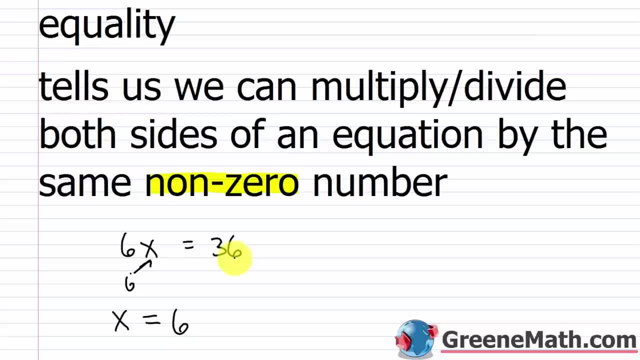 if I plug the 6 in for x there, 6 times 6 is 36. You'd have 36 equals 36. So that is correct. 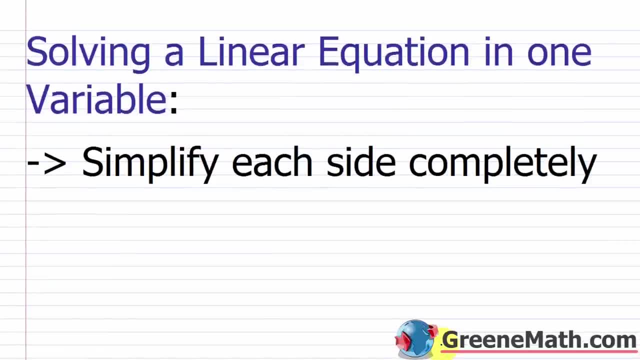 Okay, so now that we kind of have the hang of the basics, let's talk about a general procedure for solving a linear equation in one variable. And this is for any linear equation that you run across. We're going to look in the next lesson at what to do when you have fractions or decimals. But even if you didn't use that, what we're going to cover in the next lesson, you can still solve it using this procedure. All right, so the first thing you want to do is simplify each side 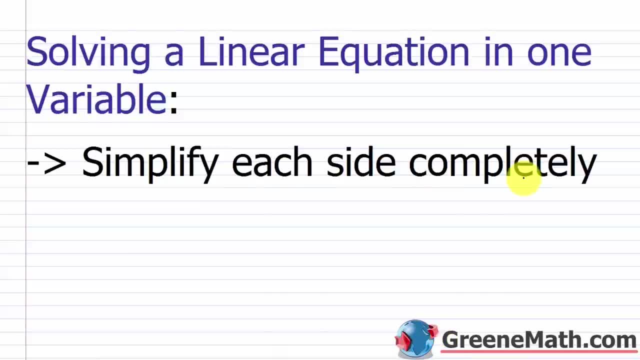 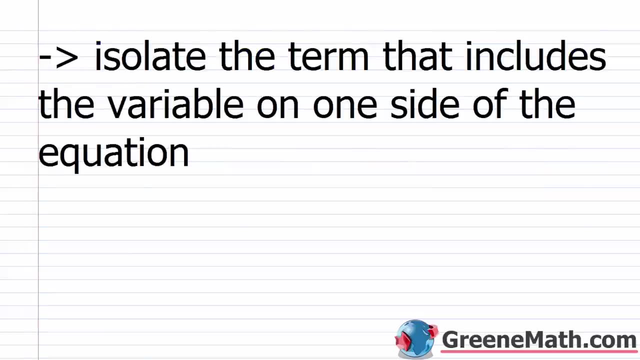 completely. So the things you're going to have to do, you are going to have to combine any like terms that you might have on each side. And you're also going to want to remove any parentheses that you have using the distributive property. All right, so the next thing you want to do is isolate the term that includes the variable on one side of the equation. So you're going to do this using the addition property of equality. So kind of think about it as, okay, I learned the addition 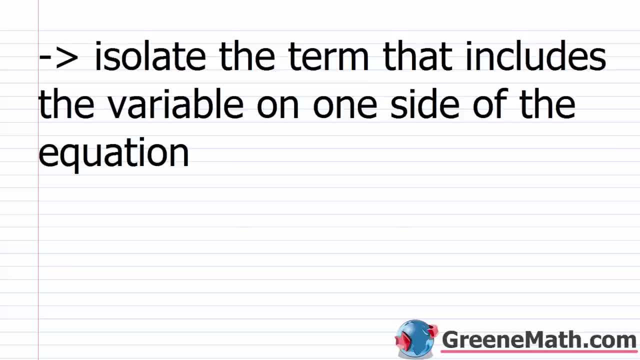 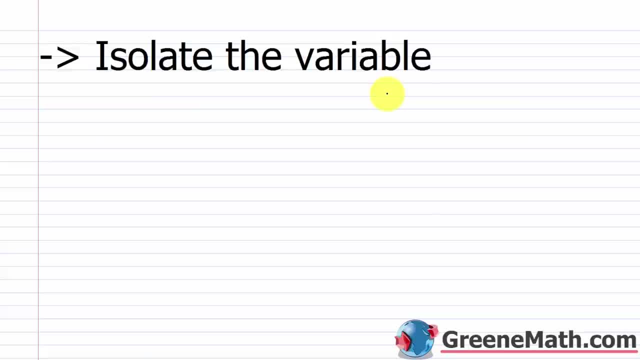 property of equality first. That's always what I'm going to use first. All right, so the next thing we're going to do is isolate the variable. And you're going to do this using the multiplication property of equality. And remember, we learned this second. So this is kind of the next step 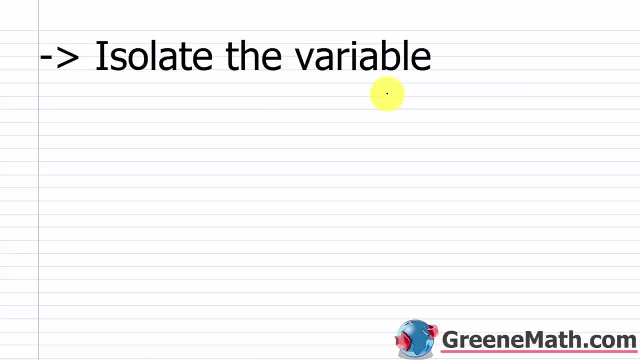 that you do. So you do the addition property of equality first. And then you're going to do the multiplication property of equality. And then the next step you do is the multiplication property of equality. Now, this is going to give you your solution. And then you just want to check the 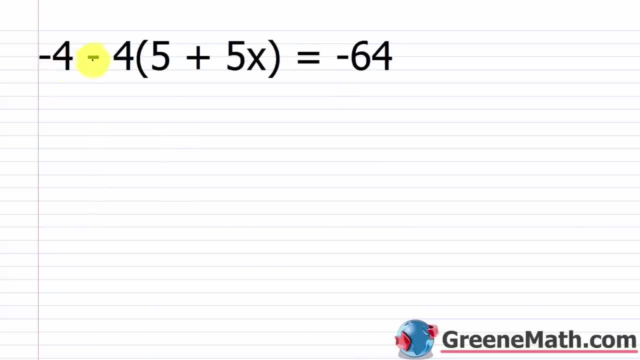 answer. All right, so let's take a look at negative four minus, we have four times the quantity, five plus five x, and this is equal to negative 64. Now, again, the first thing we want to do is simplify each side separately. So over here on the left, I have negative four. And then for the sake 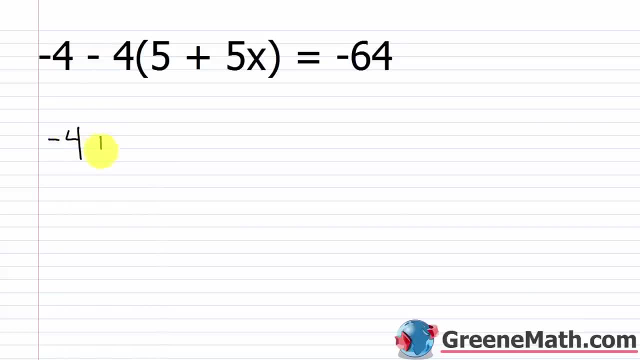 of simplicity, let's write down the number of times that we're going to have to do this. So let's write this as plus negative four times this quantity five plus five x. Because when I'm doing my multiplication here, I want to include the negative when I'm multiplying. And you don't have to write plus negative four, you can just have a minus out in front of the four and just kind of include that in the sign, right? At this point in the game, you want to do things to kind of speed up your arithmetic. All right, then this equals negative 64. 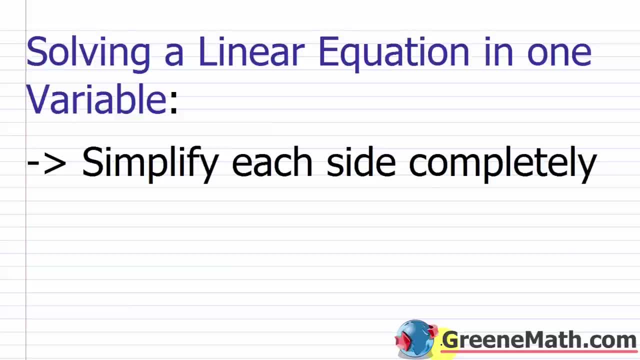 linear equation that you run across. We're going to look in the next lesson at what to do when you have fractions or decimals, But even if you didn't use that- what we're going to cover in the next lesson- you can still solve it using this procedure, All right. so the first thing you 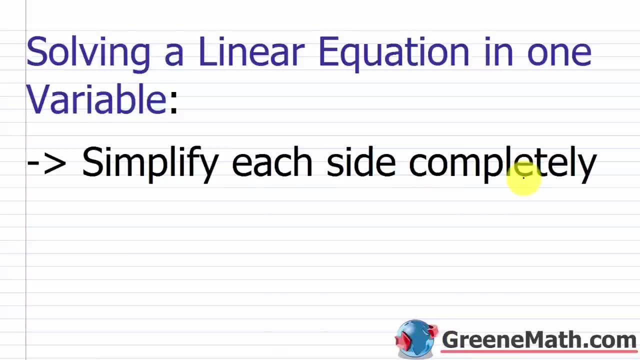 want to do is simplify each side completely. So the things you're going to have to do: you are going to have to combine any like terms that you might have on each side, And you're also going to want to remove any parentheses that you have using the distributive. 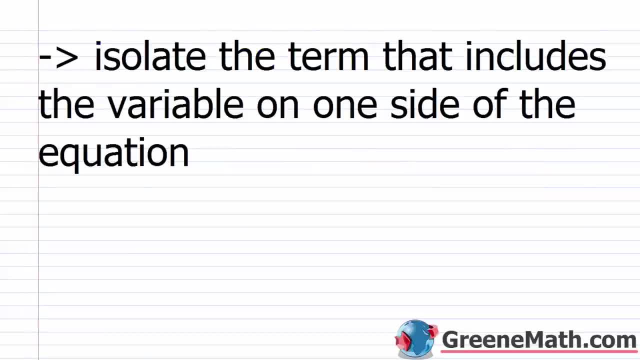 property. All right, so the next thing you have to do is isolate the term that includes the variable on one side of the equation. So you're going to do this using the addition property of equality. So kind of think about it as okay, I learned the addition property of equality first. 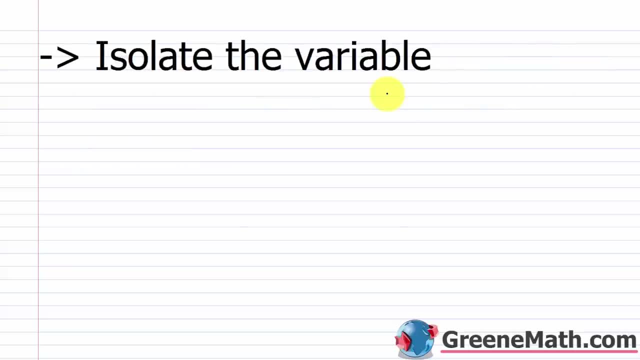 That's always what I'm going to use first. All right, so the next thing we're going to do is isolate the variable, And you're going to do this using the multiplication property of equality, And remember, we learned this second. So this is kind of the next step that you do. So you do the 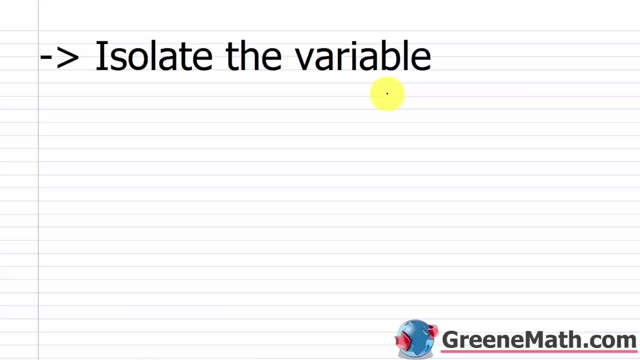 addition property of equality First, then the next step you do is the multiplication property of equality. Now, this is going to give you your solution, And then you just want to check the answer. All right, so let's take a look. at negative four minus, we have four times the quantity. 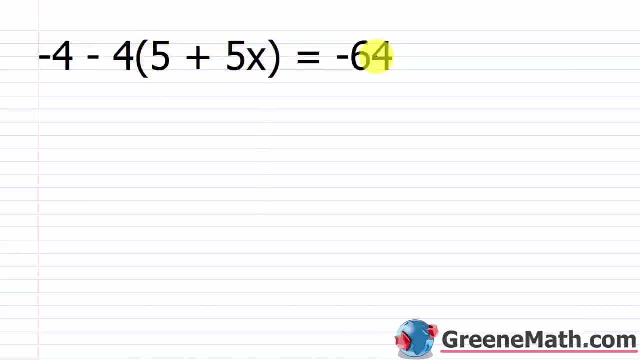 five plus five x, and this is equal to negative 64.. Now, again, the first thing we want to do is simplify each side separately. So over here on the left, I have negative four, And then, for the sake of simplicity, let's write this as plus negative four times this quantity, five plus five x, Because 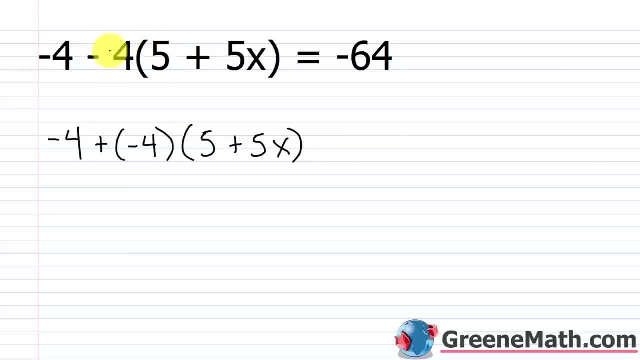 when I'm doing my multiplication. here I want to include the negative when I'm multiplying And you don't have to write plus negative four. you can just have a minus out in front of the four and just kind of include that in the sign right. At this point in the game you want to do things. 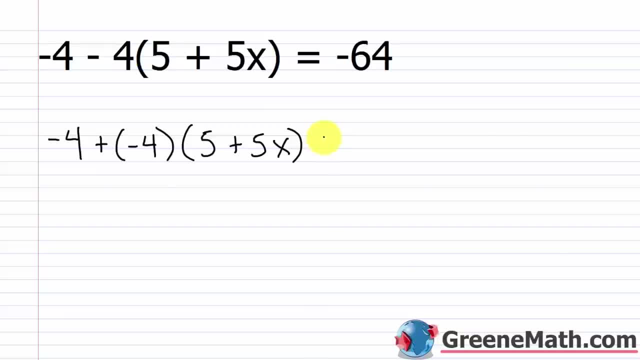 to kind of speed up your arithmetic. All right, then this equals negative 64. And then you want to nothing. I can really do with negative four at this point. I'm just going to rewrite that And then over here I'm going to use my distributive property, So I'll multiply negative. 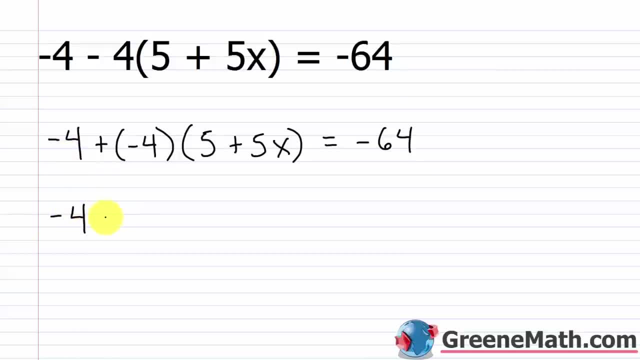 So what I can really do with negative four at this point, I'm just going to rewrite that. And then over here, I'm going to use my distributive property. So I'll multiply negative four times five, that's negative 20. So we'll have plus negative 20. Or of course, you can write minus 20 does not matter. And then I'm going to multiply by five x now. So negative four times five x would give me negative 20x. So I'm going to write minus 20x. Or of course, again, I could write plus negative 20x. Again, it doesn't matter. 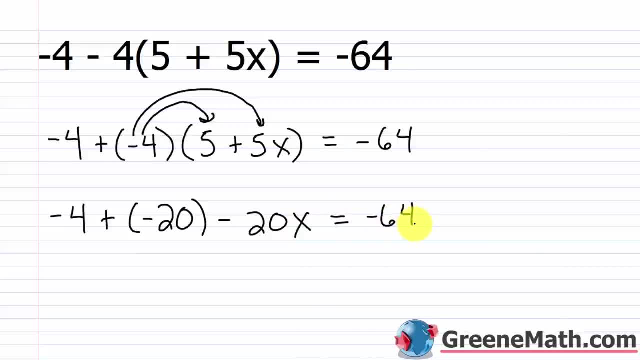 So then this equals negative 64. Now, I'm looking to combine any like terms that I have, I can't do anything with this, because I don't have any other variable term involved in this equation, right? I just have that one. But over here, I have negative four plus negative 20. 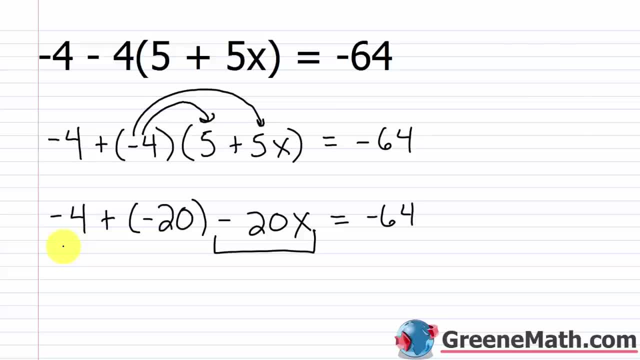 I can combine those two. So negative four plus negative 20 is negative 24. So this will be negative 24 minus 20x equals negative 64. 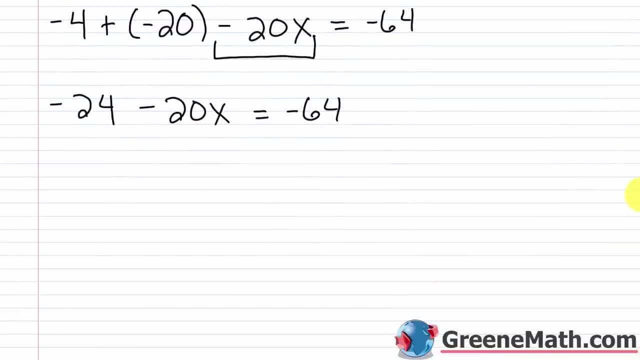 Okay, so now, I'm at the stage where I want to isolate the term that includes the variable. So that term is this right here, this minus 20x or negative 20x, however you want to think about that. So how do I isolate that? Well, we already know that we use the addition property of equality. And essentially, if I have this negative 24 over here, if I add 24 to both sides, I'm going to get rid of it, right? So if I have negative 24, I add 24. If I was to come across positive 24, I would subtract 24, right? You always want to do 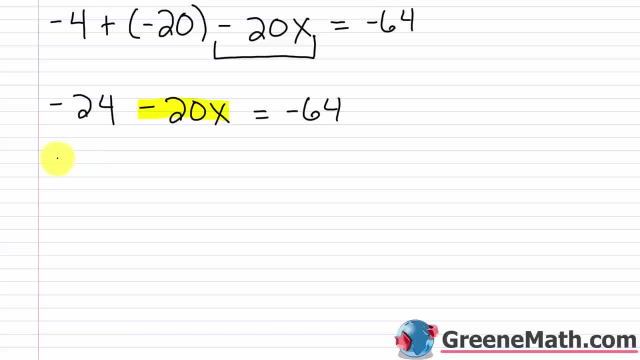 the opposite. So I'm just going to add 24 over here. And then to make that legal, I'm going to add 24 to this side of the equation. Now, this is going to cancel, right? Negative 24 plus 24 is zero. So the left side of this equation is negative 20x. On the right side, I have negative 64 plus 24. 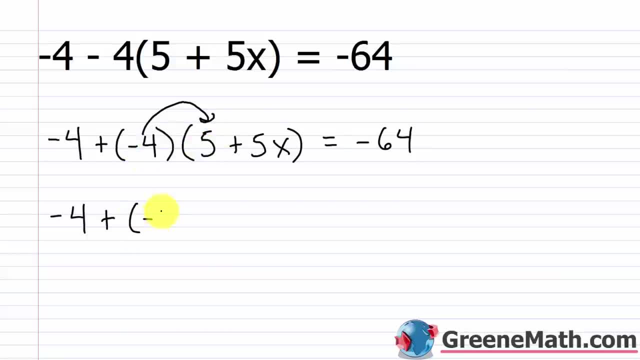 four times five, that's negative 20.. So we'll have plus negative 20.. Or of course, you can write minus 20 does not matter. And then I'm going to multiply by five x. now, So negative four times five x would give me negative 20x, So I'm going to write minus 20x. Or of course, again, I could. 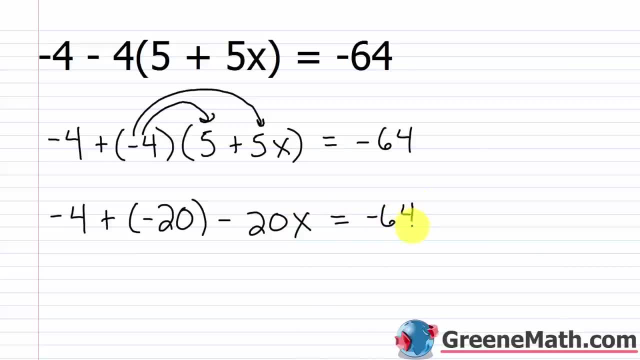 write minus 20x, but it doesn't matter. So then this equals negative 64.. Now I'm looking to combine any like terms that I have. I can't do anything with this because I don't have any other variable term involved in this equation. right, I just have that one, But over here I have negative. 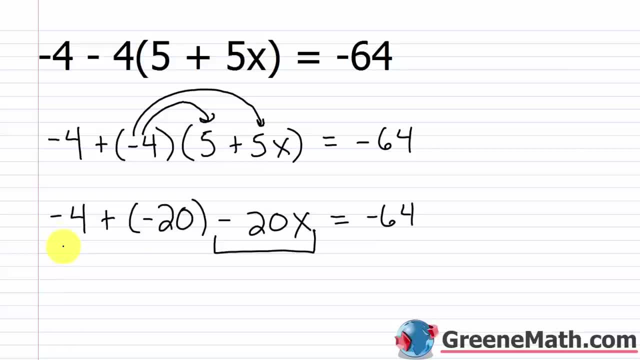 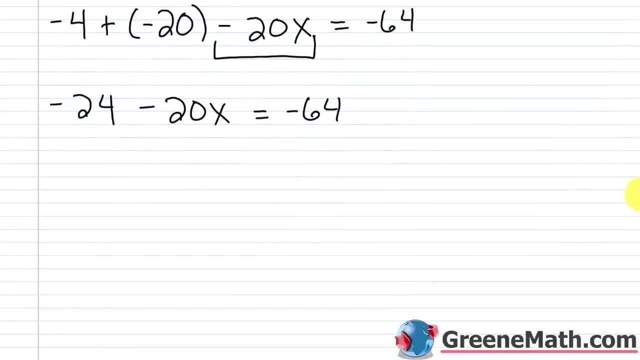 four plus negative 20.. I can combine those two, So negative four plus negative 20 is negative 24.. So this will be negative. 24 minus 20x equals negative 64.. Okay, so now I'm at the stage where I want to isolate the term. that includes: 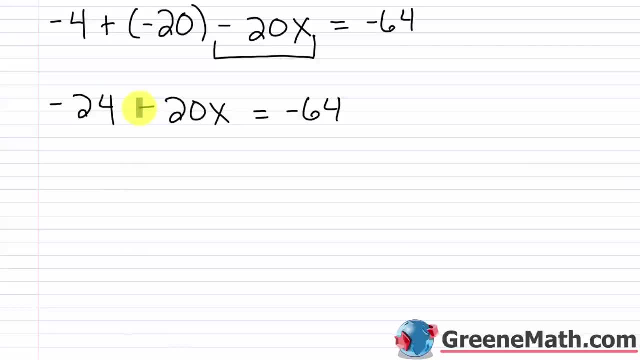 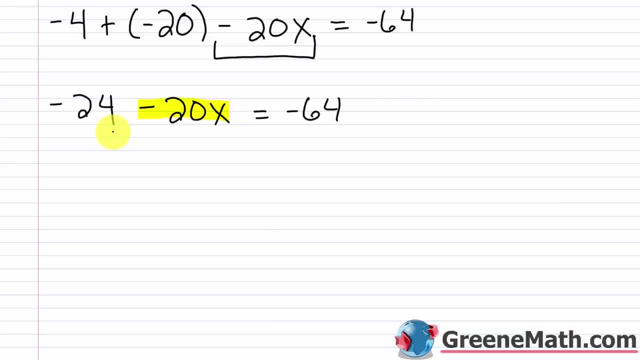 So if I have negative 24, I add 24.. If I was to come across positive 24, I would subtract 24, right, You always want to do the opposite, So I'm just going to add 24 over here And then to make. 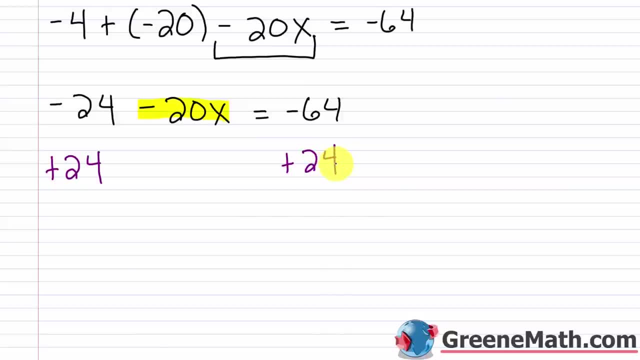 that legal. I'm going to add 24 to this side of the equation. Now this is going to cancel right. Negative 24 plus 24 is zero. So the left side of this equation is negative 20x On the right side. 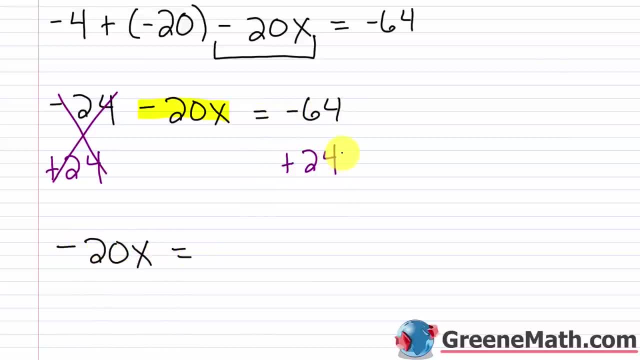 I have negative 64 plus 24.. So what's that going to be? Well, mentally we can do this. we have a four and a four here, So really I'm doing 64 minus 24, which is 40. And I'm slopping a negative on it. So this is going. 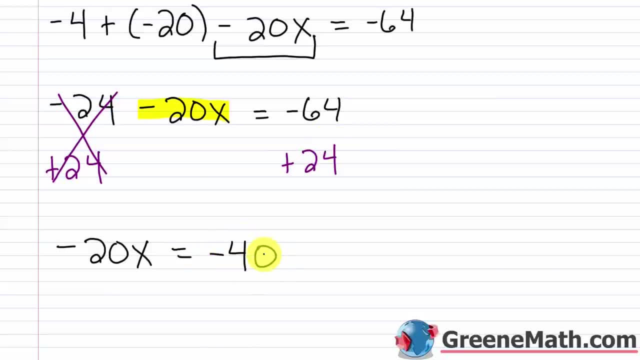 to be negative 40.. Okay, so now we're at our third step, And remember that's to isolate the variable. We do this using the multiplication property of equality. Now, if I have negative 20 times x, to get x by itself I need to divide. 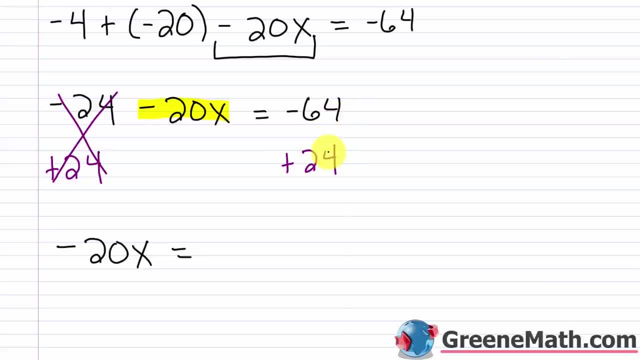 So what's that going to be? Well, mentally, we can do this. We have a four and a four here. So really, I'm doing 64 minus 24, which is 40, and I'm slopping a negative on it. So this is going to be negative 40. Okay, so now we're at our third step. And remember, that's to isolate the variable. We do this using the multiplication property of equality. Now, if I have negative 20 times x, to get x by itself, I need to divide, right? Remember, this is multiplication, the opposite of that would be division, I need to divide by negative 20. Again, just look at what's being done to x. If negative 20 is multiplied by x, the opposite of multiplication is division. Okay, so if I'm multiplying negative 20 by x, I divide by negative 20, so that these two will cancel out and become one, and I just have x by itself. Now, because I do it to this side, I must also do it to this side. 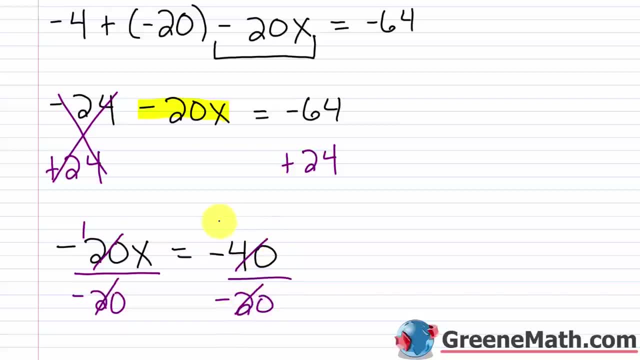 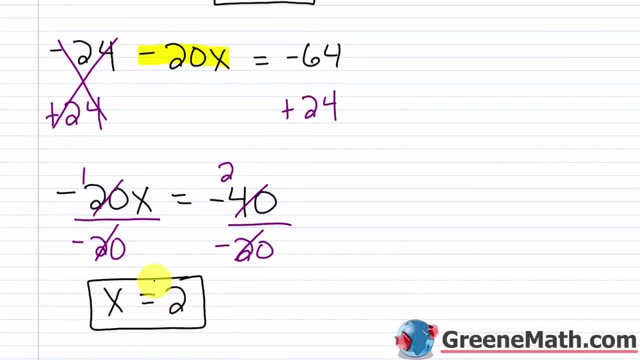 And negative 40 divided by negative 20 would give me two. So what I get as my solution is that x is equal to two. All right, so we definitely want to check this and make sure we got the right answer. So let me erase everything. And we'll go back up to the top. All right, 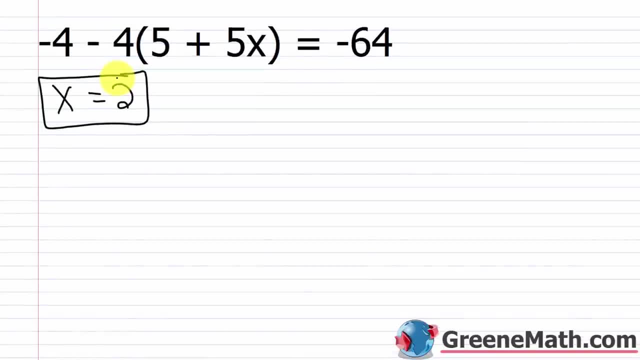 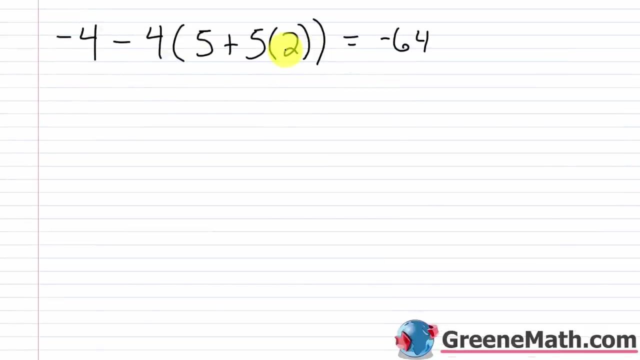 so we have x equals two, we have negative four, we have negative four, minus four times a quantity five, where I see the x, I'm going to plug in a two, and then close the parentheses and then equals negative 64. Okay, let's crank this out, we're going to start out inside the parentheses here. And we're gonna start out with five times two, five times two is 10. And if I add 10 to five, 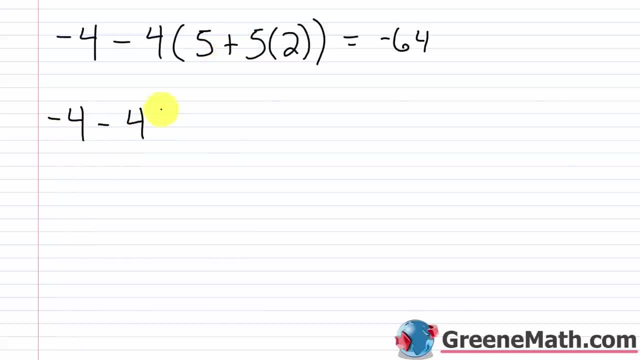 I'd have 15. So I'll have negative four, minus four times 15. And this should equal negative 64. So I'm going to do multiplication first. So you can think about this as negative four times positive 15. That would give me negative 60. So negative four, minus 60 equals negative 64. And of course, it does right negative four minus 60 is negative 64. So we get negative 64. On the left, we have 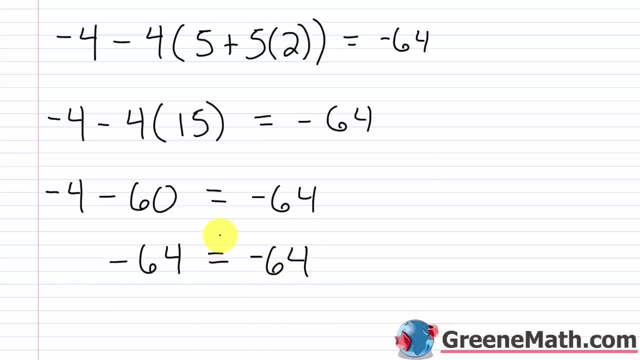 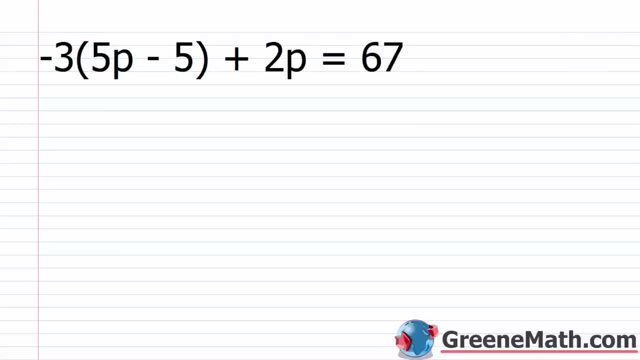 negative 64 on the right. And so yes, x equals two is the correct solution. All right, let's take a look at another one. We have negative three times the quantity five p minus five plus two p equals 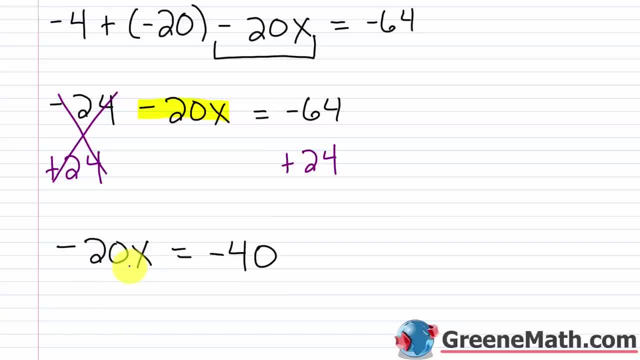 right, remember, this is multiplication. the opposite of that would be division. I need to divide by negative 20.. Again, just look at what's being done to x. If negative 20 is multiplied by x, the opposite of multiplication is division. Okay, so if I'm multiplying negative, 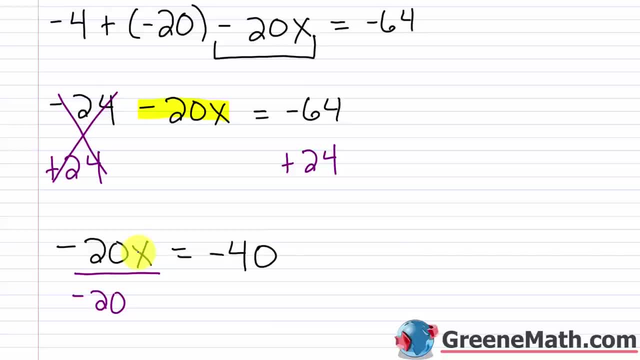 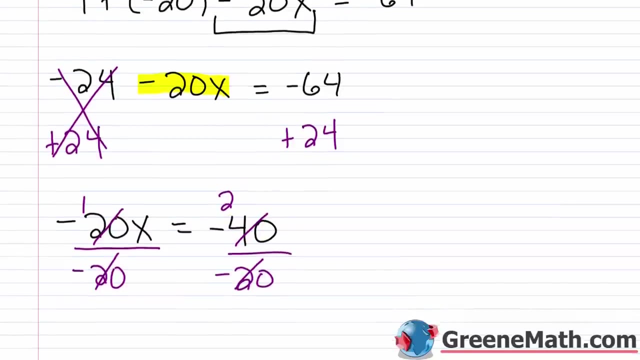 20 by x, I divide by negative 20, so that these two will cancel out and become one and I just have x by itself. Now, because I do it to this side, I must also do it to this side, And negative 40 divided by negative 20 would give me two. So what I get as my solution? 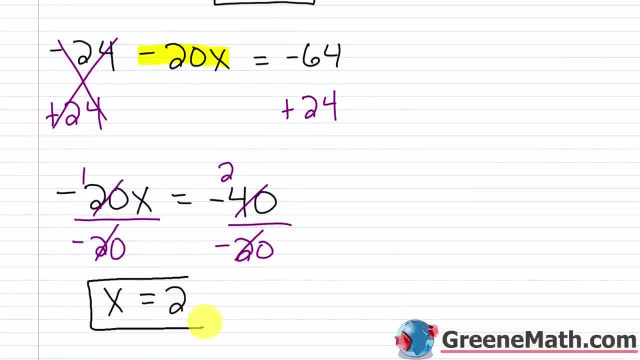 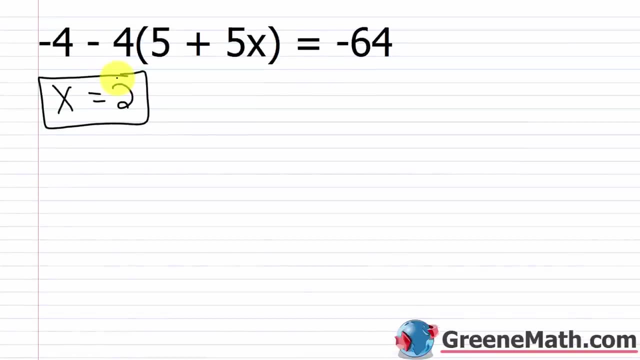 is that x is equal to two. All right, so we definitely want to check this and make sure we got the right answer. So let me erase everything And we'll go back up to the top. All right, so we have x equals two. we have negative four. we have negative four minus four times the quantity. 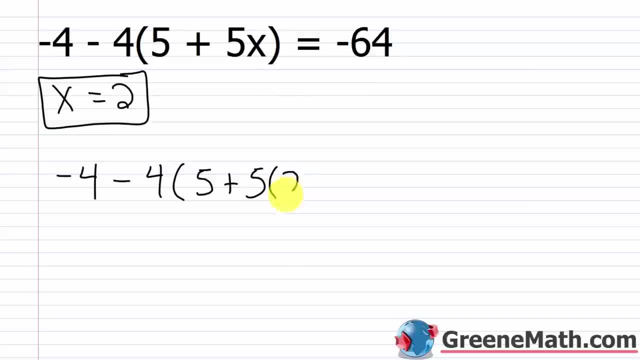 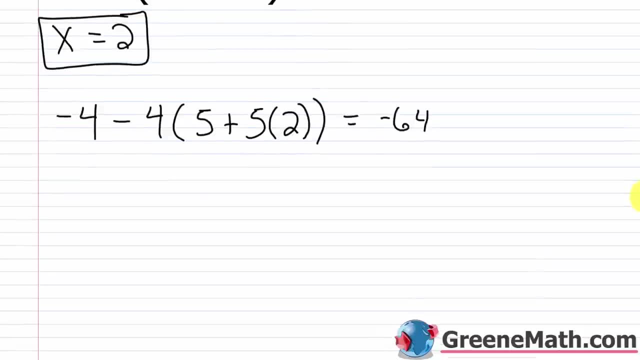 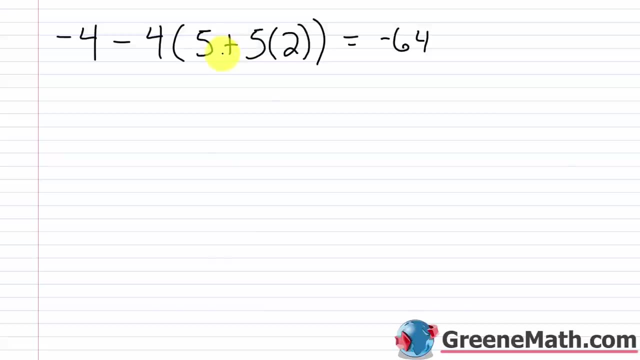 five plus five, where I see the x, I'm going to plug in a two and then close the parentheses and then equals negative 64.. Okay, let's crank this out. we're going to start out inside the parentheses here And we're gonna start out with five times two. five times two is 10.. And if I add 10 to five, 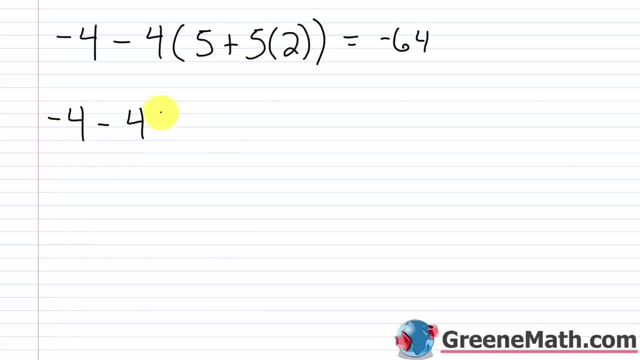 I'd have 15.. So I'll have negative four minus four times 15.. And this should equal negative 64.. So I'm going to do multiplication first, So you can think about this as negative four times positive 15, that will give me negative 60. So negative four minus 60 equals negative 64.. 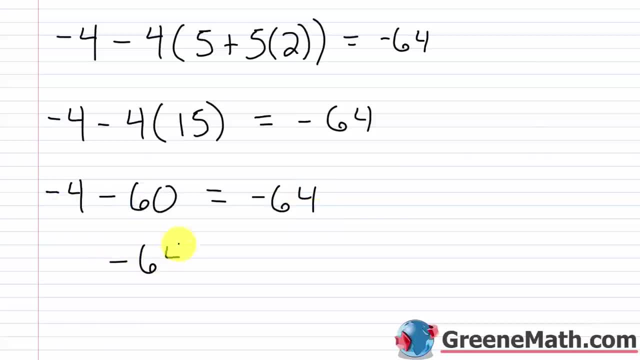 And of course it does right. Negative four minus 60 is negative 64. So we get negative 64 on the left, we have negative 64 on the right, And so, yes, x equals two is the correct solution. All right, let's take a look at another one. We have negative three times the quantity. 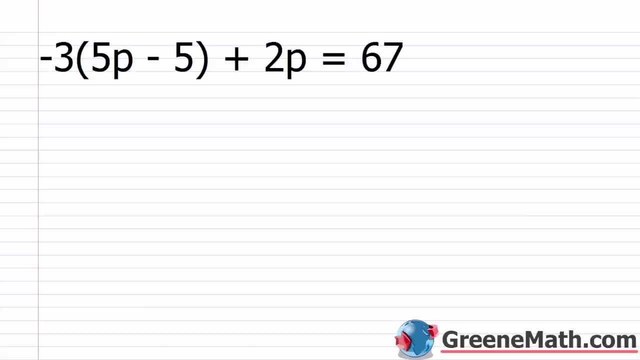 five p minus five plus two p equals 67. So again, the first thing I want to do is simplify each side separately. So to do that over here, I'm going to use my distributive property, I'm going to multiply negative three times five P. 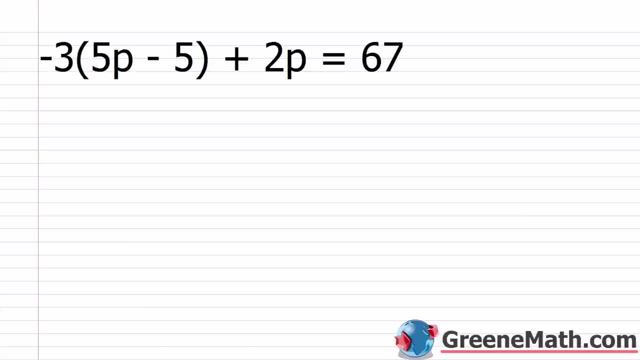 67. So again, the first one is negative 64. And the second one is negative 64. And the third one is negative 64. So the first thing I want to do is simplify each side separately. So to do that over 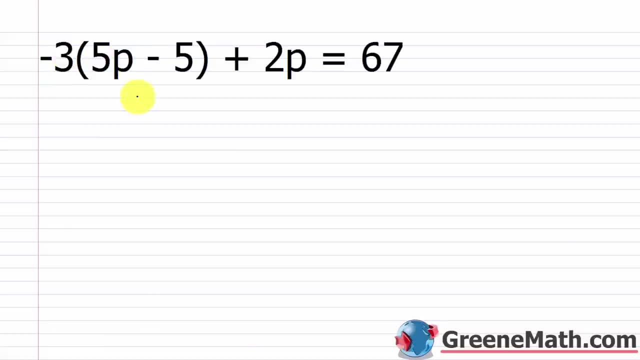 here, I'm going to use my distributive property, I'm going to multiply negative three times five p, that's going to give me negative 15 p. And then next, I'm going to multiply negative three times negative five. So negative three times negative five is positive 15. And then plus two p equals 67. 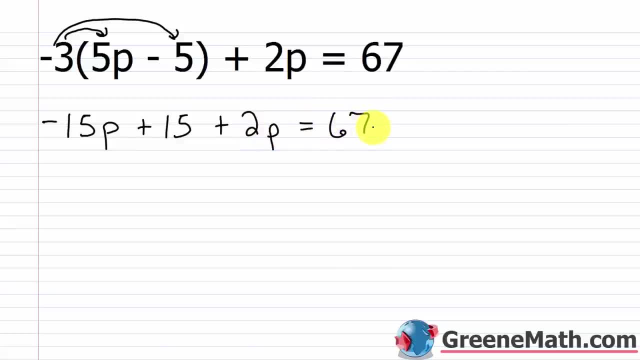 All right, now I want to combine any like terms that I have. So over here, I have negative 15 p, and I have two p. So negative 15 plus two is negative 13. The variable comes along for the ride. So this is negative 13 p plus 15 equals 67. There's nothing 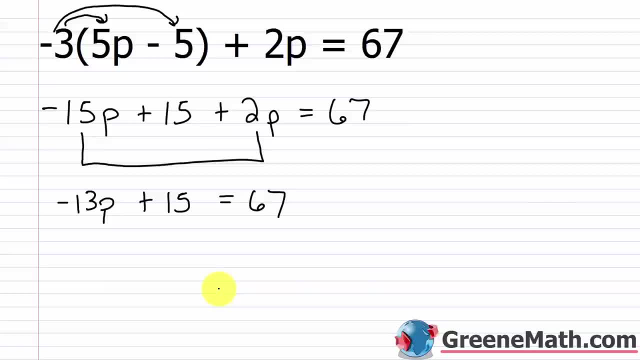 else to simplify on each side. And so now I move on to the next step where I'm going to isolate the variable term on one side of the equation. Now, if I look at my variable term, it's negative 13 p. What's being done to it? Well, I'm adding this 15 right here. So in order to isolate negative 13 p, I need to do the opposite operation, I need to subtract 15 away, where you think about it as adding negative 15 to both sides, right? So I need to subtract 15 over here. And then over here to make it legal, I need to also subtract 15. So this is going to cancel and become zero. And I have isolated my variable term on one side. And then I'm going to add negative 15 to both sides. And so I have negative 13 p here. And then over here, 67 minus 15, that's going to give me 52, right? 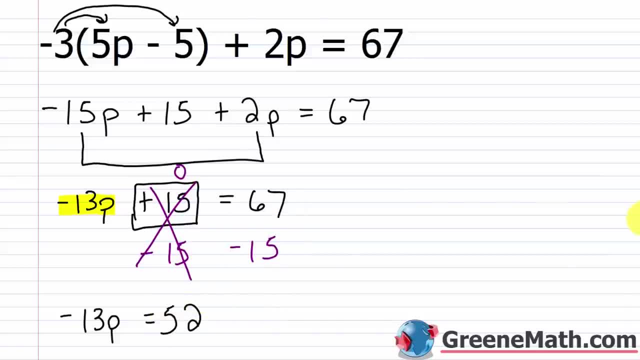 Seven minus five is two, six minus one is five. All right. So now what's left, we want to isolate 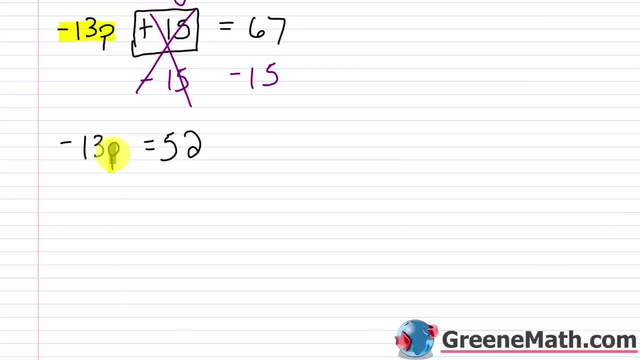 the variable, right? So we want to isolate p. And how do we do that? Well, we always want to look at what's being done to that variable, right? So in this case, we have negative 13, that's multiplying our variable p. So to undo multiplication, we do that by multiplying our variable p. 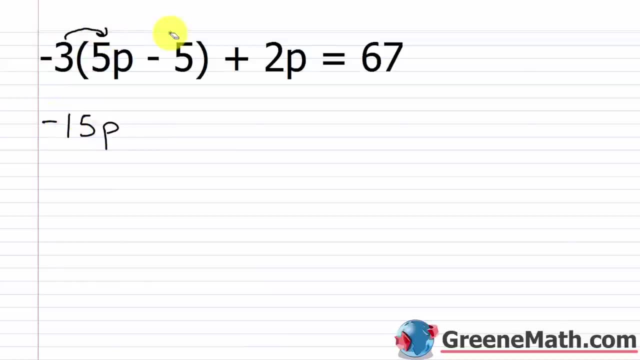 And that's going to give me negative 15 p. And then next I'm going to multiply: negative three times negative five. So negative three times negative five is positive 15.. And then plus two p equals 67.. Alright, now I want to combine. 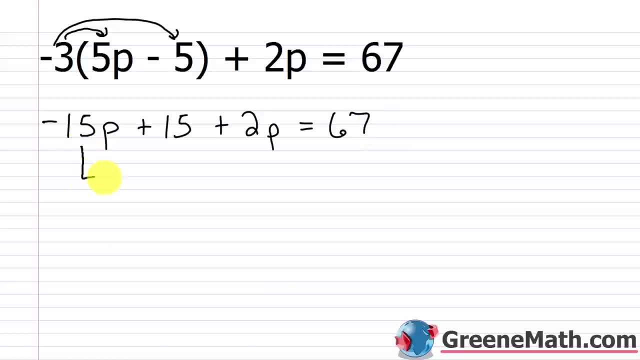 any like terms that I have. So over here I have negative 15p and I have 2p, So negative 15 plus 2 is negative 13.. The variable comes along for the ride. So this is negative. 13p plus 15 equals 67.. 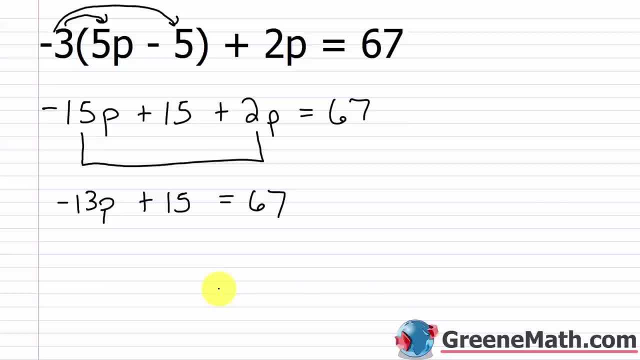 There's nothing else to simplify on each side, And so now I move on to the next step, where I'm going to isolate the variable term on one side of the equation. Now, if I look at my variable term, it's negative 13p. What's being done to it? Well, I'm adding this 15 right here. 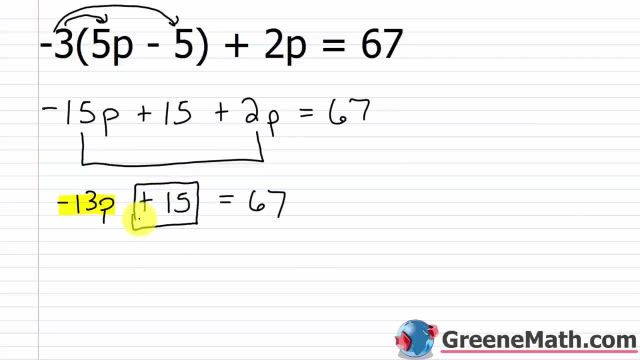 So, in order to isolate negative 13p, I need to do the opposite operation. I need to subtract 15 away where you think about it as adding negative 15 to both sides, right. So I need to subtract 15 over here and then, over here, to make it legal, I need to also subtract 15.. So this is going to 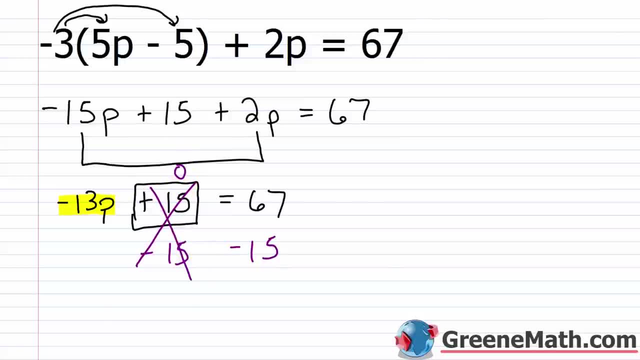 cancel and become zero And I have isolated 15p. So I need to do the opposite operation. I need to add negative 15 to both sides, My variable term on one side. So I have negative 13p here And then over here 67 minus 15.. 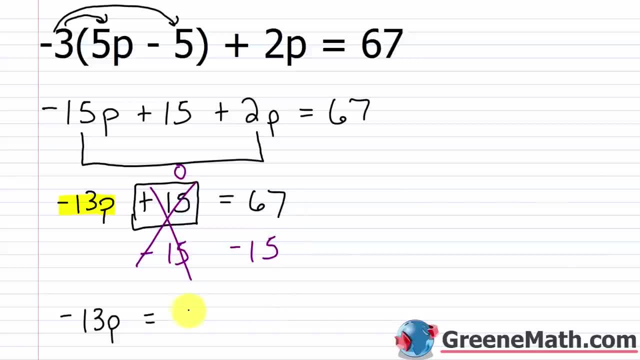 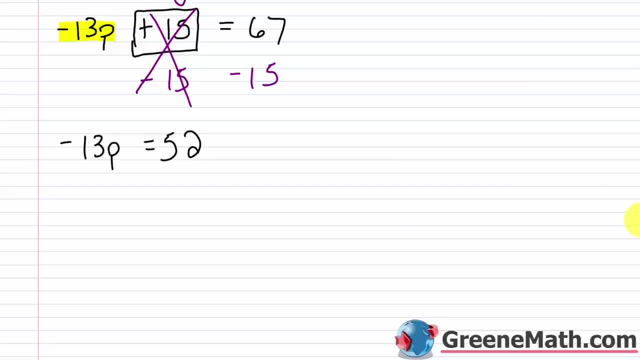 That's going to give me 52, right, 7 minus 5 is 2.. 6 minus 1 is 5.. All right, So now what's left? we want to isolate the variable right. So we want to isolate p. And how do we do that? Well, 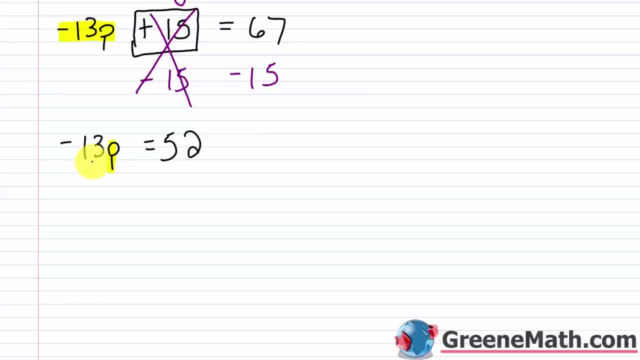 we always want to look at what's being done to that variable right. So in this case we have negative 13. That's multiplying our variable p. So to undo multiplication we do division right, So we're going to divide both sides of. 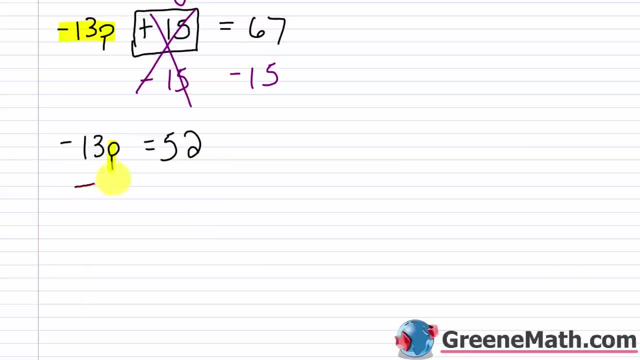 the equation by the coefficient of p, which is negative 13.. Very, very simple. So this cancels with this And I'm just going to have p. And then, over here, what is 52 divided by negative 13?? Well, it's going to give me negative 4.. And that's my solution: p is going to equal negative. 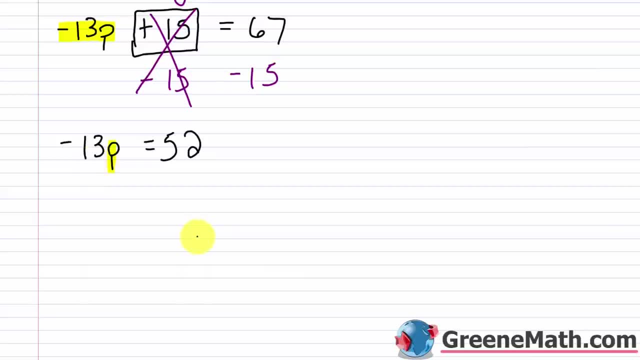 All right, so we're going to divide both sides of the equation by the coefficient of p, which is negative 13. Very, very simple. So this cancels with this, and I'm just going to have p. And then over here, what is 52 divided by negative 13? Well, it's going to give me negative four. 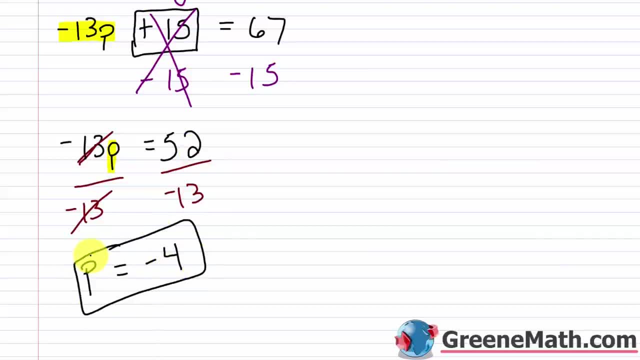 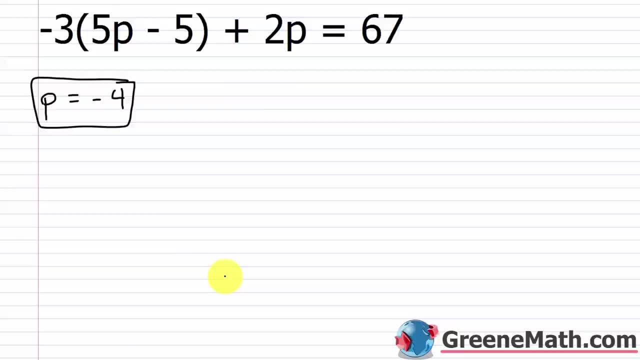 And that's my solution. p is going to equal negative four. All right, let me erase everything, and then we're going to go back and check. All right, so let's see if we got the right answer. We're going to have negative three times, inside the parentheses, we have five, plug in a negative four for p. So times negative four minus five, close the parentheses, plus two times negative four equals 67. So we're going to start out inside the parentheses here. We always multiply first. Five times negative four is negative 20. Negative 20 minus five is negative 25. So this would be negative three. 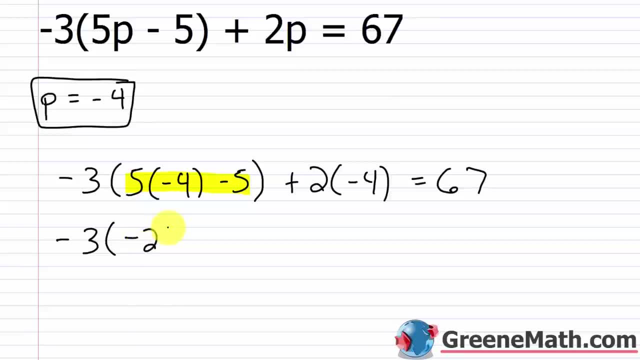 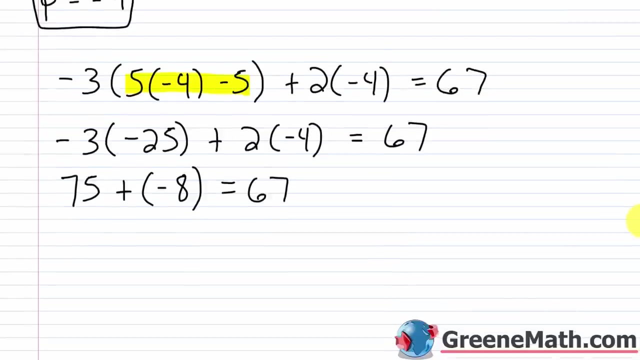 Negative three times negative 25, plus we have two times negative four equals 67. So we're going to multiply before we add. Negative three times negative 25 is 75, plus we have two times negative four, that's negative eight. And this equals 67. All right, so what is 75 plus negative eight, or what is 75 minus eight? Well, that's going to be 67. So we have 67 equals 67. And so p equals negative four 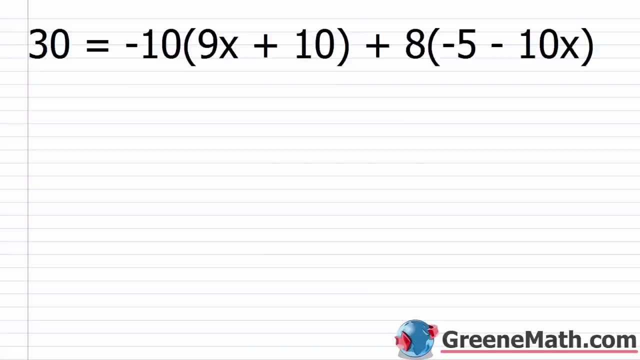 is the correct solution. All right, let's take a look at another one. We have 30 equals negative 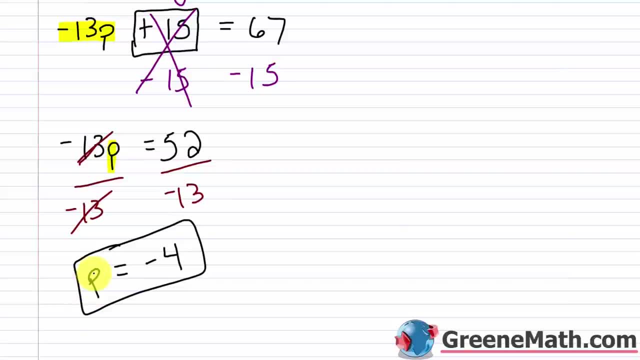 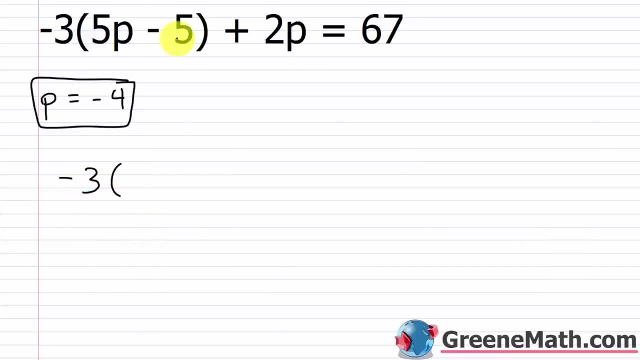 4. And that's my solution. So I'm going to divide both sides of the equation by the coefficient of 4.. All right, Let me erase everything and then we're going to go back and check. All right, So let's see if we got the right answer. We're going to have negative 3 times inside the parentheses. 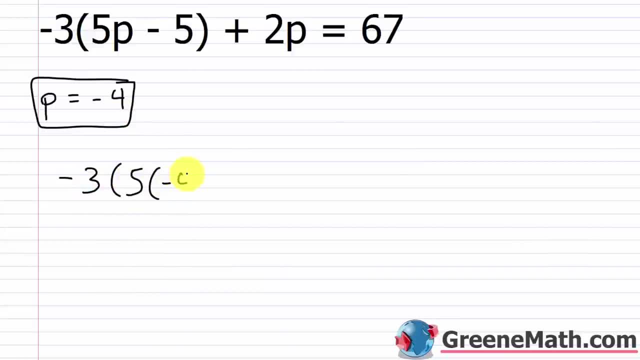 we have 5, plug in a negative 4 for p. So times negative 4, minus 5, close the parentheses. plus 2 times negative 4 equals 67. So we're going to start out inside the parentheses here. 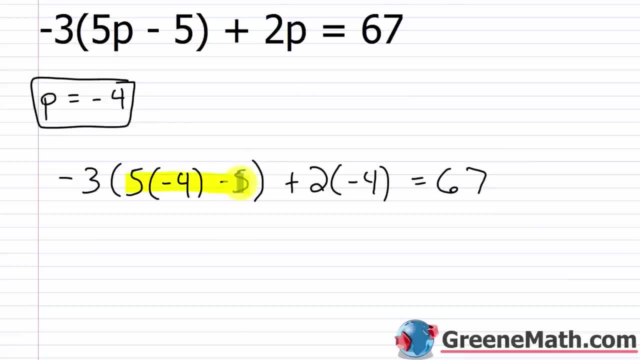 We always multiply first: 5 times negative 4 is negative 20.. Negative 20 minus 5 is negative 20,, 5.. So this would be negative 3, negative 3 times negative 25, plus we have 2 times negative 4. 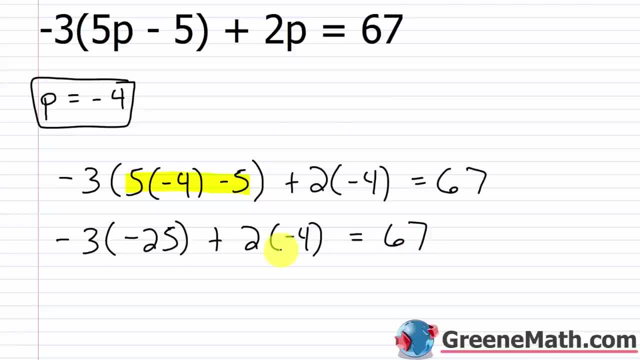 equals 67.. So we're going to multiply before we add Negative. 3 times negative, 25 is 75, plus we have 2 times negative 4, that's negative 8. And this equals 67.. All right, So what is 75?? 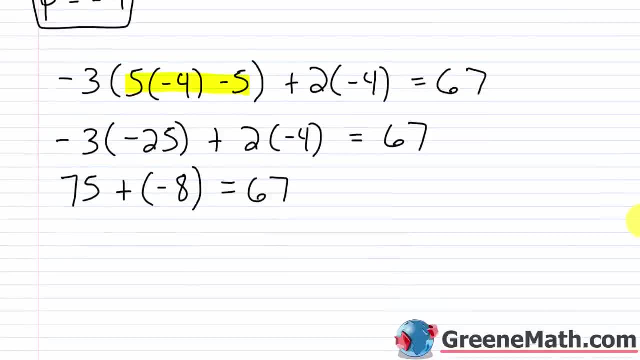 75 plus negative 8, or what is 75 minus 8?? Well, that's going to be 67. So we have 67 equals 67. And so p equals negative 4 is the correct solution. All right, Let's take a look at another one. 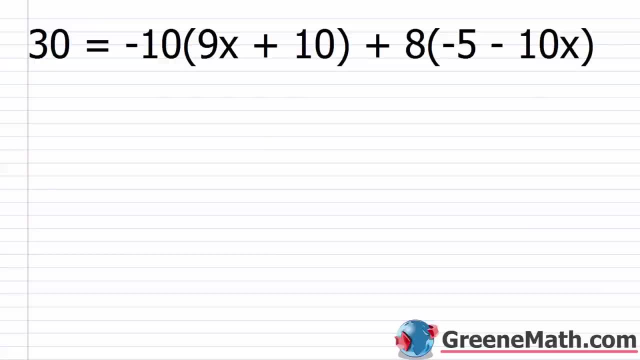 We have 30 equals negative 10 times the quantity 9x plus 10,, plus 8 times the quantity negative 5 minus 10x. So again, I want to simplify each side separately. So I have 30 on the left. 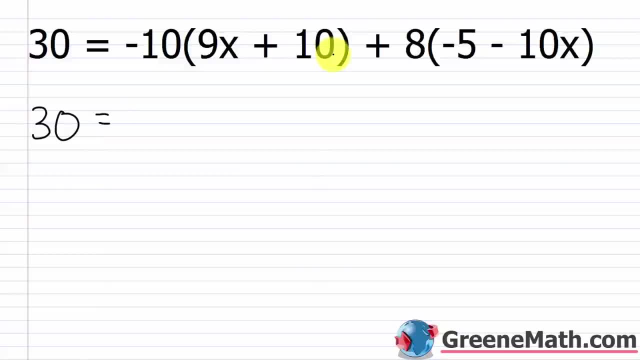 nothing I can really do with that. On the right, I'm going to use my distributive property and I'm going to multiply negative 10 times 9x, So that's going to be negative 90x. plus I'm going to have negative 10 times positive 10, which is negative 100. So I can write plus. 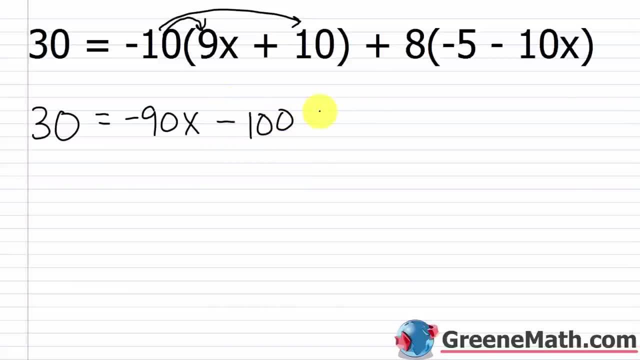 negative 100, or I can just write minus 100. So then plus now, we have 8 times negative 5, that's going to be negative 40. So I'm just going to write minus 40. And then we have 8 times. 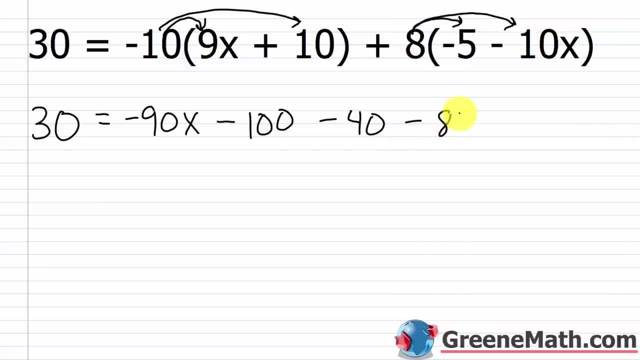 negative 10 times the quantity, negative 5.. So that's going to be negative 40.. So I'm just going to write 9x and that's going to be negative 80x. All right, So now we want to combine like terms. 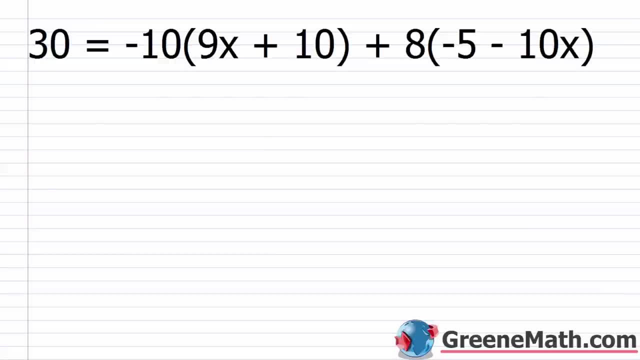 10 times the quantity 9x plus 10, plus eight times the quantity negative five minus 10x. So again, I want to simplify each side separately. So I have 30 on the left, nothing I can really do with that. On the right, I have 30 plus negative four, that's negative 10. And so I have 30 plus negative four minus 10. So I'm just going to write negative 10 times negative 5, which is minus 40. And on the right, I'm going to use my distributive property. And I'm going to multiply negative 10 times 9x. So that's going to be negative 90x. Plus I'm going to have negative 10 times positive 10, which is negative 100. So I can write plus negative 100, I can just write minus 100. So then, plus, now we have eight times negative 5, that's going to be negative 40. So I'm just going to write minus 40. And then we have eight times negative 10x. And that's going to be negative 50.ан �斮 10x. Ant x Will be eld 8 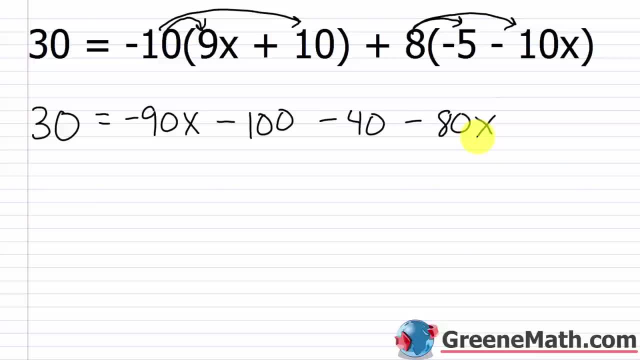 80 x all right so now we want to combine like terms and basically you can see that we have negative 90 x and we have negative 80 x those can be combined and we also have negative 100 and we have negative 40 those can be combined as well so we have 30 on the left that's not changing on the right negative 90 x minus 80 x or negative 90 x plus negative 80 x however you want to think about that that's going to give me negative 170 x then i'm going to have negative 100 minus 40 that's minus 140 so now that we've simplified each side completely meaning i can't do anything else to either side to make it more simple i'm going to isolate the variable term so in this 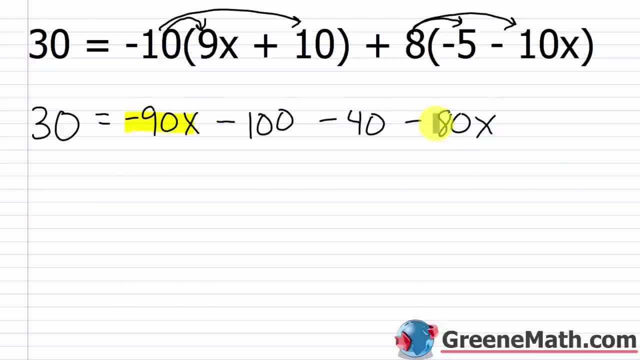 And basically you can see that we have negative 90x and we have negative 80x. those can be combined. And we also have negative 100. And we have negative 40. Those can be combined as well. So we have 30 on the left, that's not changing. On the right: negative 90x minus 80x or negative. 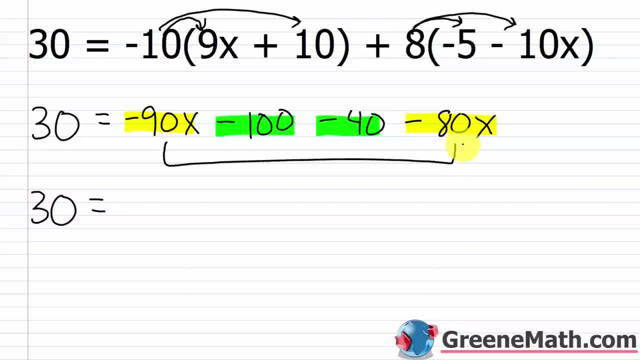 90x plus negative 80x. However you want to think about that, that's going to give me negative 170x. Then I'm going to have negative 100 minus 40, that's minus 140.. So now that we've simplified. 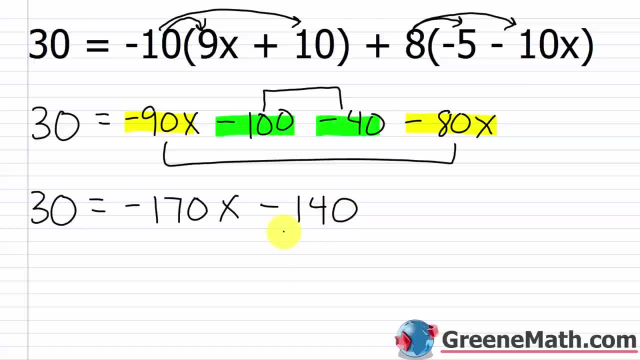 each side completely, meaning I can't do anything else to either side. to make it more simple, I'm going to isolate the variable term. So in this case that's going to be this right here, this negative 170x, Again, again, again. What can we do here to isolate that? We have to look at what's being. 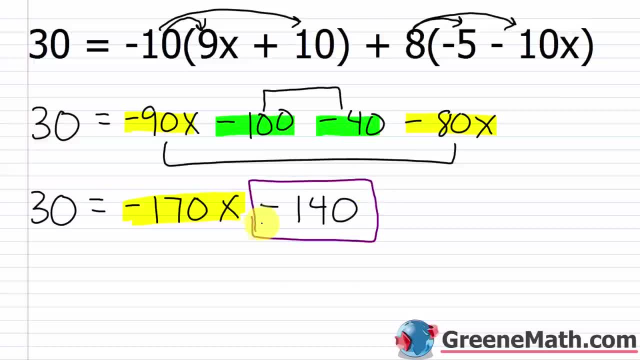 done to the variable term, I'm subtracting away 140.. So if I'm subtracting away 140, again always look to add the opposite. So the opposite of negative 140 is positive 140. And I got to do it to both sides to make this legal, So that cancels becomes zero. 30 plus 140 is 170. 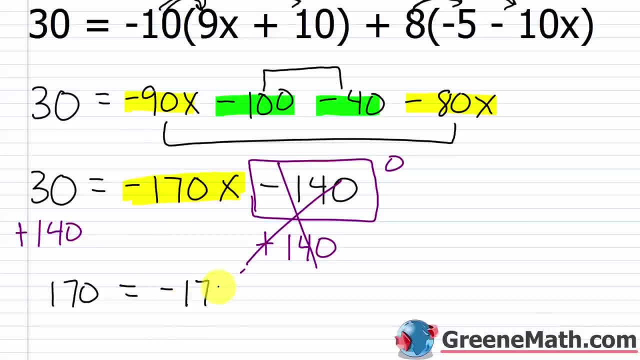 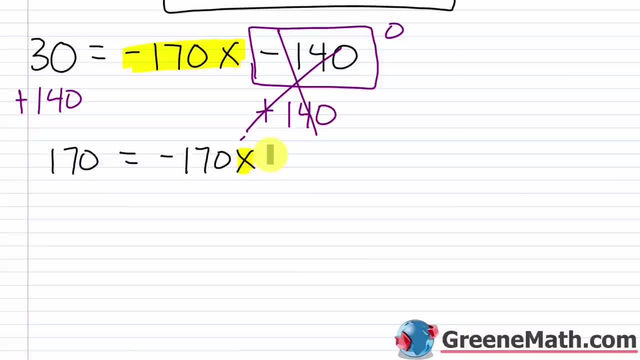 So this equals over here, just 140.. And then I'm going to add the opposite. So I'm going to add the negative 170x And to get x by itself, to isolate the variable, which is our next step. we look at what's being done to x And in this case we have multiplication. So again, 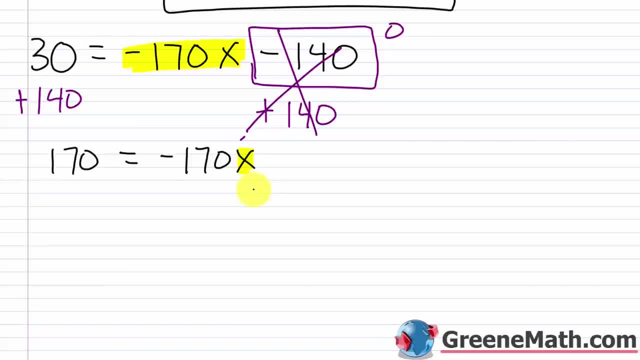 you always look to do the opposite. If you're multiplying, you divide. If you're dividing, you multiply. If you're adding, you subtract. So it's just that simple. So in this case, we have multiplication, So we look to division. So divide this by the coefficient of x, which is 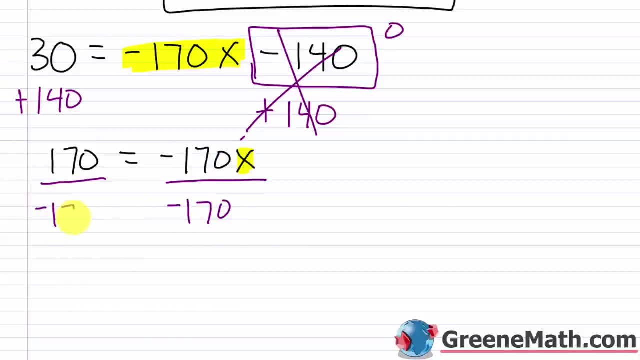 negative 107.. Divide this by negative 170.. So this and this are going to cancel and become 1.. 1 times x is just x. And then over here, 170 divided by negative 170 is negative 1.. So you have: negative 1 equals x. 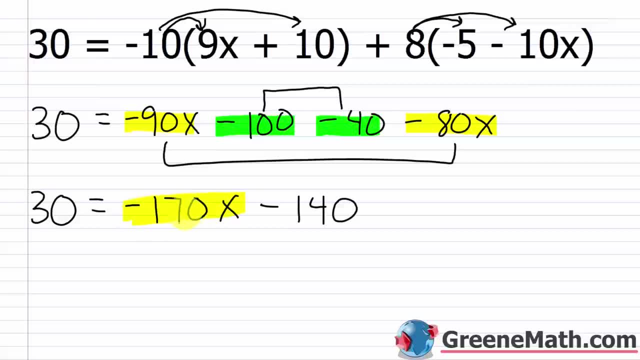 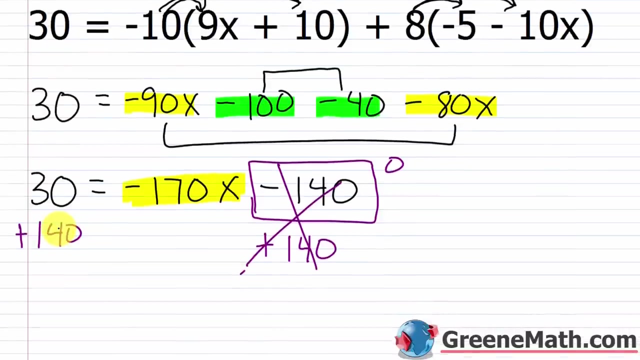 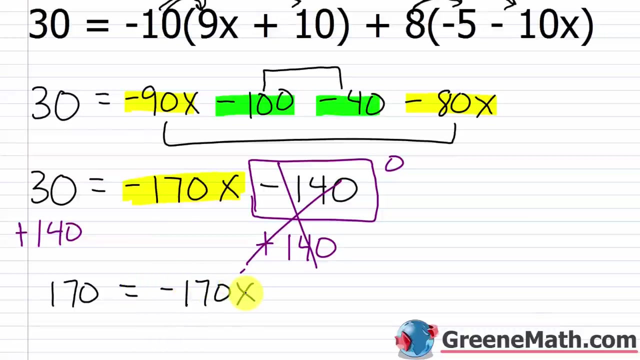 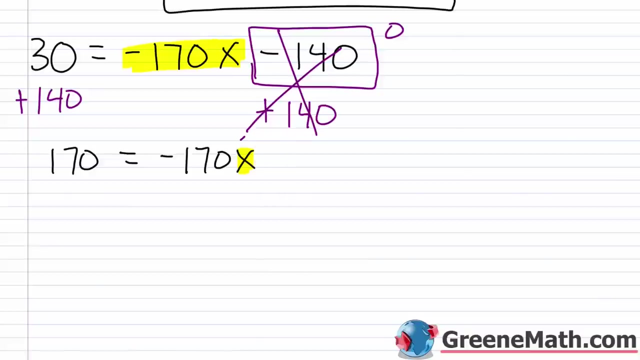 case that's going to be this right here this negative 170 x now again again again what can we do here to isolate that we have to look at what's being done to the variable term i'm subtracting away 140 so if i'm subtracting away 140 again always look to add the opposite so the opposite of negative 140 is positive 140 and i got to do it to both sides to make this legal so that cancels becomes zero 30 plus 140 is 170 so this equals over here just negative 170 x and to get x by itself to isolate the variable which is our next step we look at what's being done to x and in this case we have multiplication so again you always look to do the opposite if you're multiplying you divide if you're dividing you multiply if you're adding you're subtracting so it's it's just that simple so in this case we have multiplication so we look to division so divide this by the coefficient of x which is negative 107 divide this by negative 170 so this and this are going to cancel and become one one times x is just x and then over here 170 divided by negative 170 is negative one so you have negative one equals x or you can flip that a lot of people like to have the variable on the left myself included so if i see 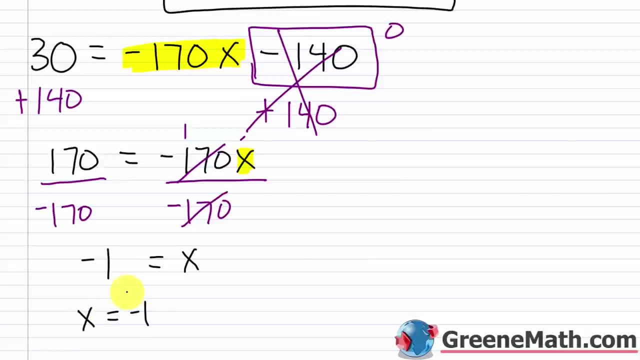 something like this i just kind of flip it and say okay well x equals negative one it doesn't really matter these two mean the exact same thing right it does not matter whatsoever 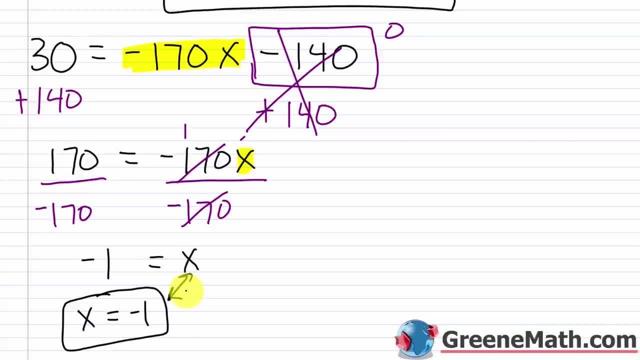 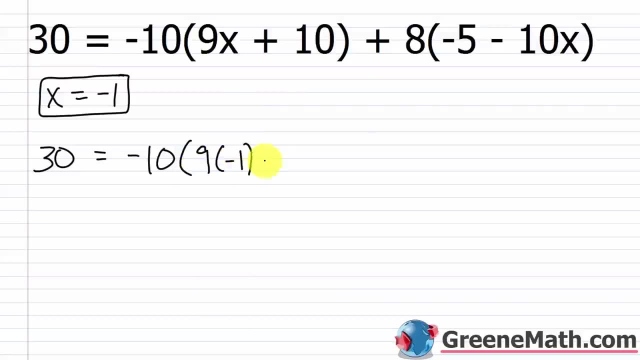 all right so let's erase everything and check our answer all right so we have 30 equals negative 10 times this quantity 9 times negative 1 plus 10 then plus 8 times negative 5 minus 10 times negative 1 and then close parentheses okay so we have 30 over here on the left and then equals inside the parentheses here 9 times negative 1 is negative 9 negative 9 plus 10 is negative 9 is 1 so i would have negative 10 times 1 which is just negative 10 right we don't even need to kind of write that then plus we have 8 times and then we have inside of here negative 5 minus 10 times negative 1 so i can just think about this as negative 10 times negative 1 that's going to 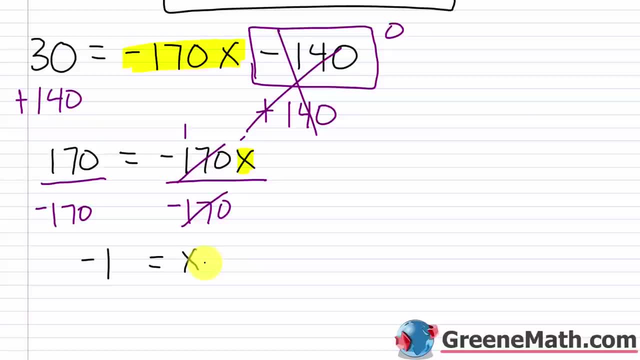 or you can flip that. A lot of people like to have the variable on the left, myself included. So if I see something like this, I just kind of flip it and say, okay, well, x equals negative 1.. It doesn't really matter. These two mean the exact same thing, right? It does not. 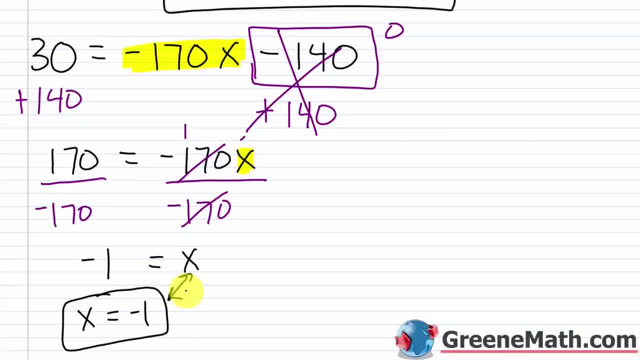 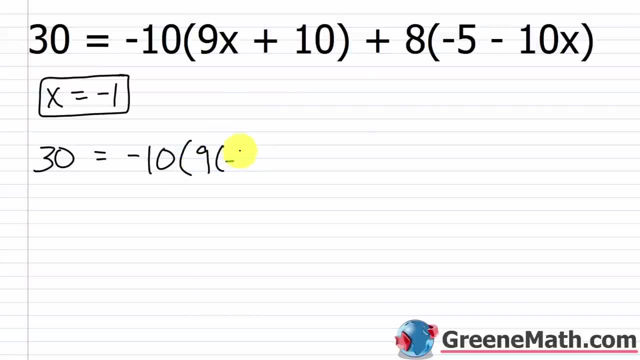 matter whatsoever. All right, So let's erase everything and check our answer. All right, So we have 30 equals negative 10 times this quantity, 9 times negative, 1 plus 10, then plus 8 times negative 5 minus 10 times negative 1, and then close parentheses. Okay, So we have 30 over here. 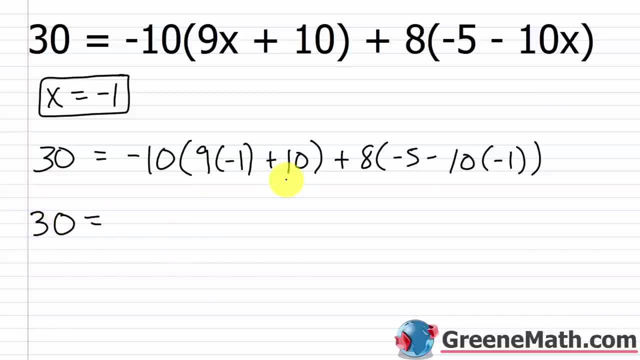 on the left and then equals inside of the parentheses. here: 9 times negative, 1 is negative 9, negative 9 plus 10. Is 1.. So I would have negative 10 times 1, which is just negative 10, right, We don't even need to. 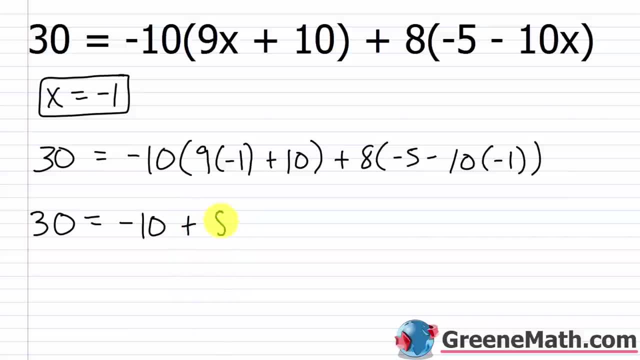 kind of write that Then plus we have 8 times and then we have inside of here negative 5 minus 10 times negative 1. So I can just think about this as negative 10 times negative 1. That's going to be positive 10.. So negative 5 plus 10 would be 5.. So I'd have 8 times 5 here. 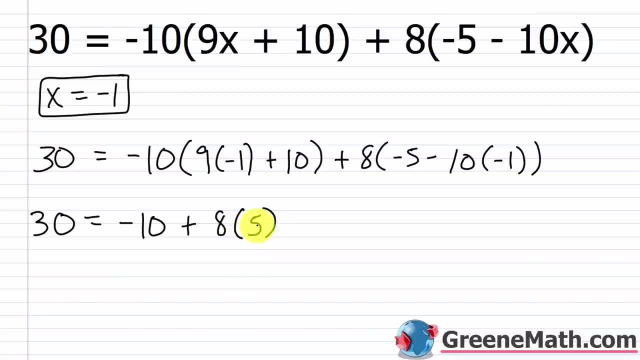 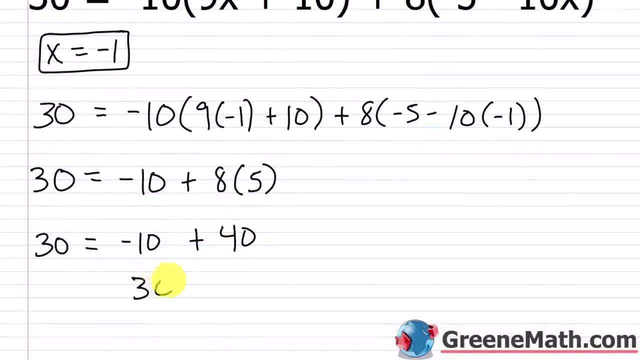 Now, in this next step, I would do my multiplication: 8 times 5 is 40. And so now negative 10 plus 40 would be 30.. So I'd have 30 equals 30. And so my solution: 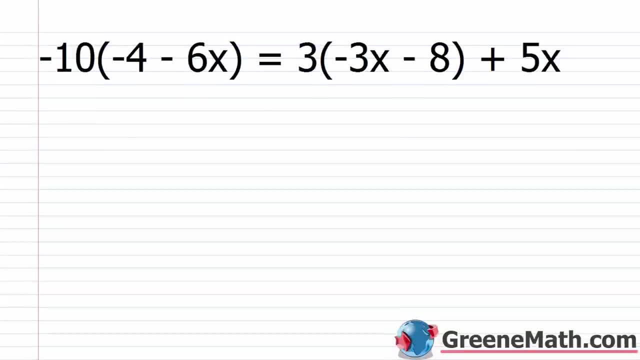 x equals negative 1 is correct. Okay, Let's take a look at one final problem. So we have negative 10 times the quantity negative. 4 minus 6x. This is equal to 3 times the quantity negative: 3x minus 8, then plus 5x. All right, So we're going. 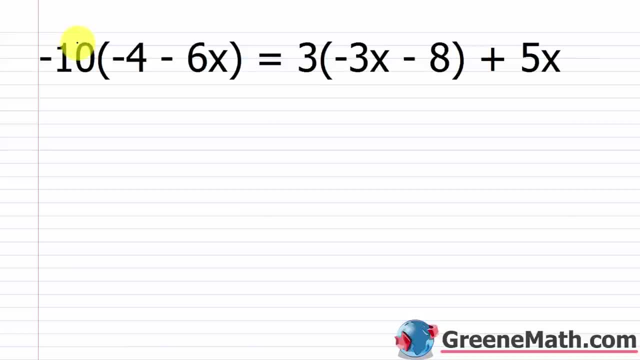 to start by again simplifying each side separately. So on the left: negative 10 times. negative 4 is 40. Then negative 10 times. think about this as negative 6x, That's going to be plus 60x, And this equals over here 3 times. negative 3x is negative 9x, And then 3 times. 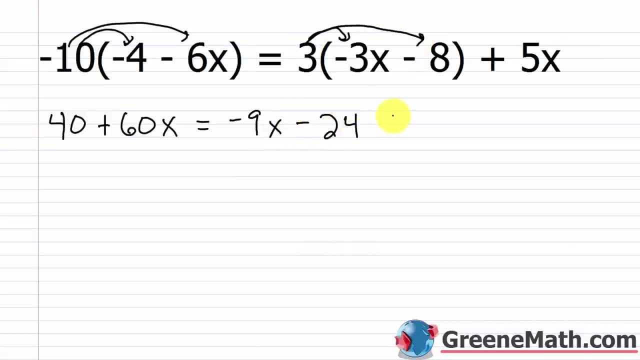 negative 8 is 9x And then negative 10 times negative 6x is negative 9x, And then negative 8x is negative 24.. So minus 24 plus 5x, Okay, So now I want to combine like terms. Nothing I can combine. 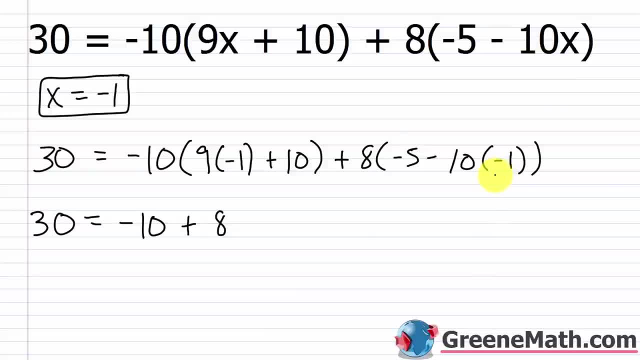 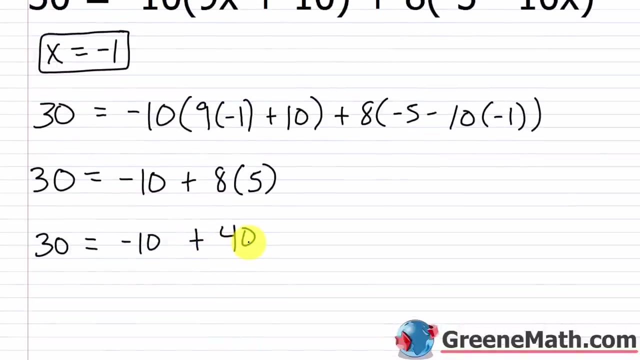 be positive 10 so negative 5 plus 10 would be 5 so i'd have 8 times 5 here now in this next step i would do my multiplication 8 times 5 is 40 and so now negative 10 plus 40 would be 30 so i'd have 30 equals 30 and so my solution x equals 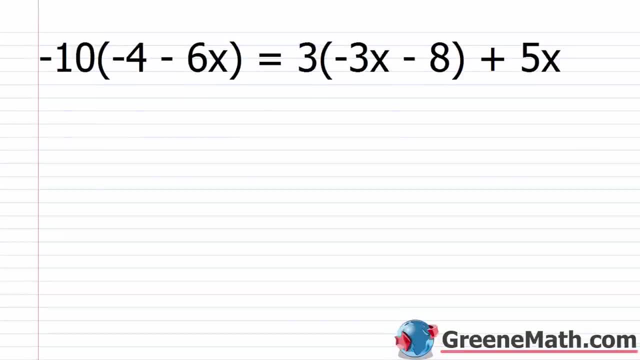 negative 1 is correct okay let's take a look at one final problem so we have negative 10 times the quantity negative 4 minus 6x this is equal to 3 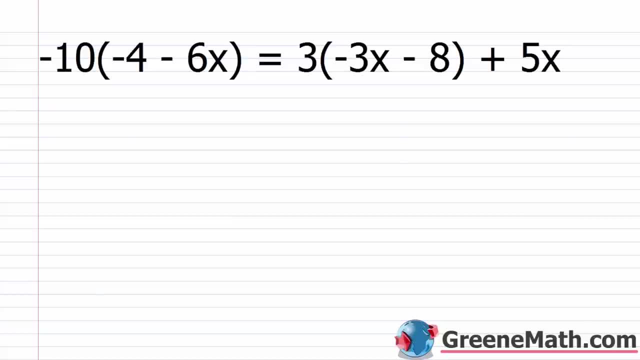 times the quantity negative 3x minus 8 then plus 5x all right so we're going to start by again simplifying each side separately so on the left negative 10 times negative 4 is 40 then negative 10 times think about this as negative 6x that's going to be plus 60x and this equals over here 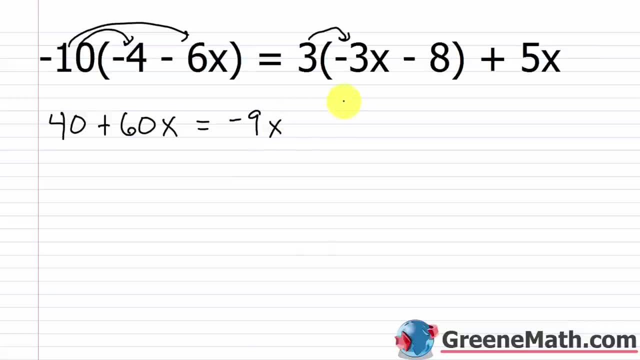 3 times negative 3x is negative 9x and then 3 times negative 8 is negative 24 so minus 24 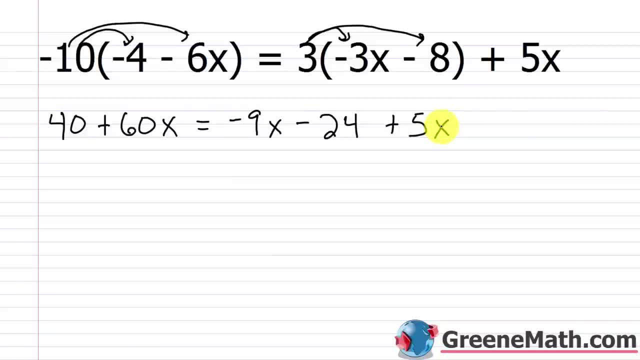 plus 5x okay so now i want to combine like terms nothing i can combine on the left on the right i can combine the negative 9x and the 5x that's going to give me negative 4x so i'm going to write this as 40 plus 60x equals again this will be negative 4x when i add negative 9x and 5x 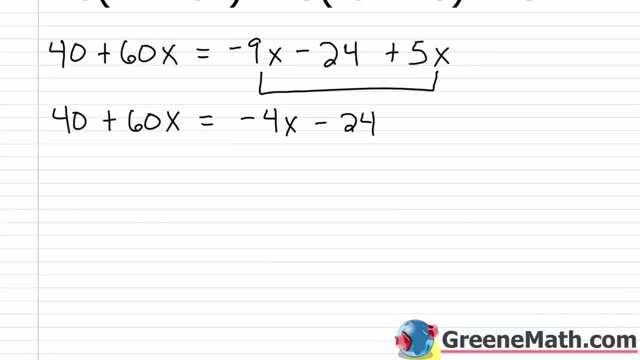 minus 24 all right so i want all the variable terms on one side of the equation that's how i kind of isolate the variable term on one side and i have 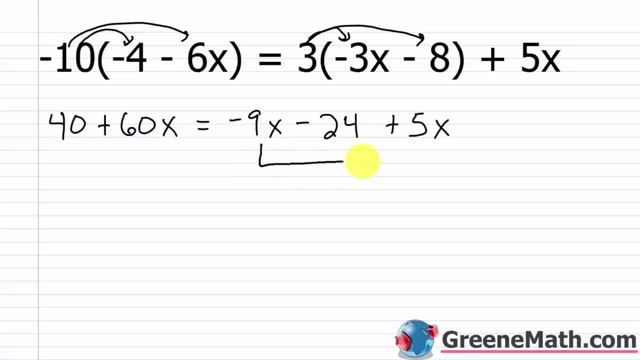 on the left, On the right, I can combine the negative 9x and the 5x. That's going to give me negative 4x. So I'm going to write this as 40 plus 60x equals again this will be negative 4x. 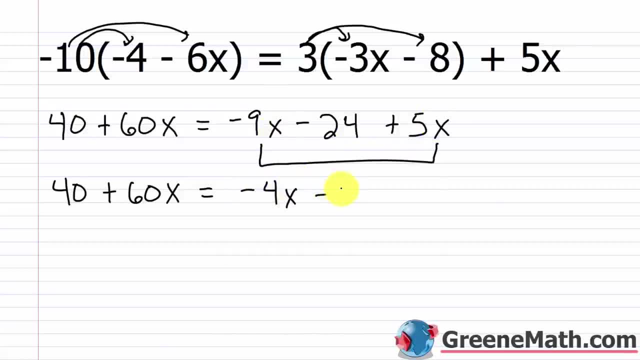 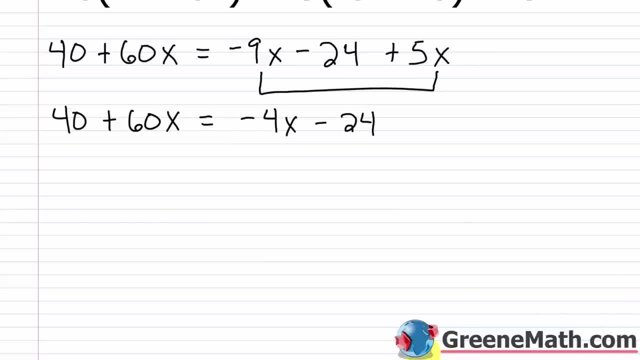 when I add negative 9x and 5x minus 24.. All right, So I want all the variable terms on one side of the equation. That's how I kind of isolate the variable term on one side and I have just a number on the other. So in the previous examples it's been kind of easy to do that. Here what? 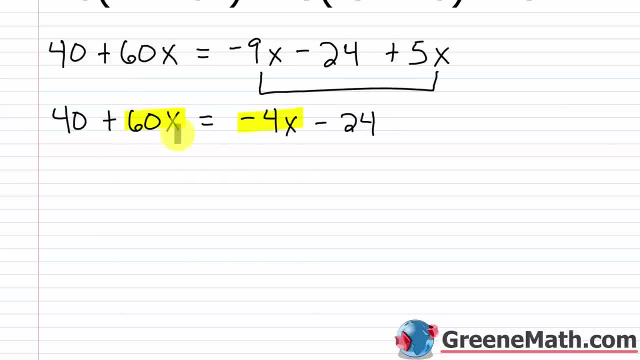 you're going to notice is that you have a variable term here and here. Now what you want to do is use the addition property of equality to get both on one side. Remember, I can move anything. So if I have negative 4x over here, I can just. 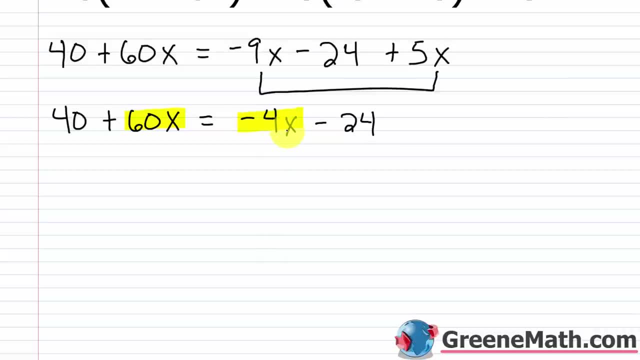 add 4x and make it disappear on this side, but I have to do the same thing over here to make it legal. So in other words, if I add 4x here, it's going to disappear on this side. Negative 4x plus. 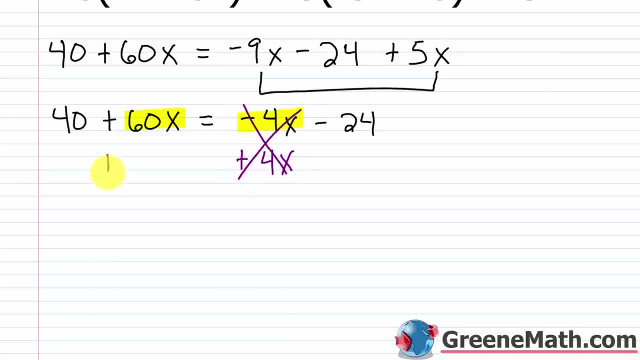 4x. that's zero, So it's gone, But it reappears over here because I have to also do it on this side to make it legal. So now I'll have 40 plus 60x. plus 4x is 64x, and this equals negative 24.. This is still not what I want. 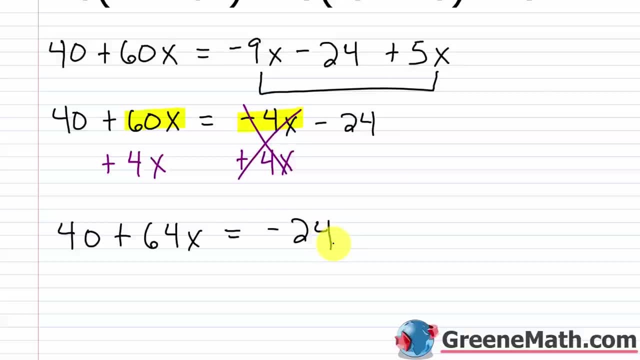 because I want a variable term on one side of the equation and I want just a number on the other. So, in order to do this again, if I'm adding 40 to the variable term, 64x to make this 40 go away. 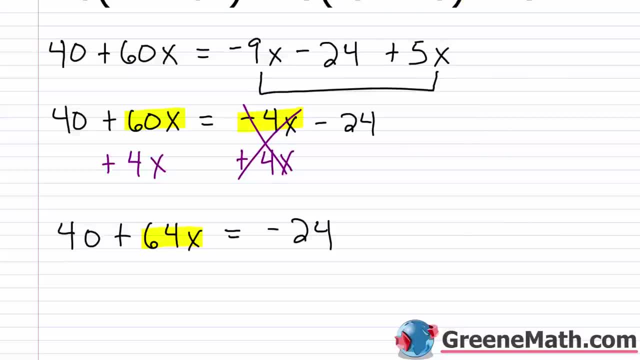 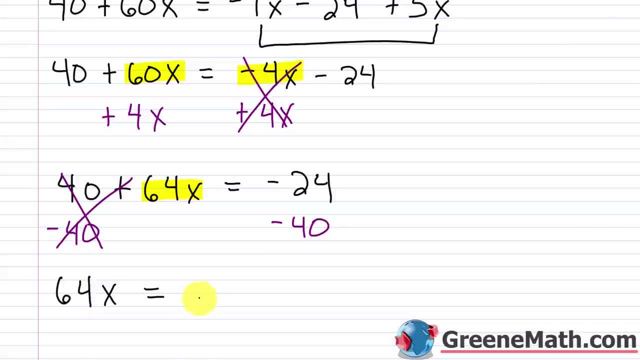 I'm just going to subtract it away, right, But I have to do it to both sides, That's the key. So minus 40 over here and minus 40 over here. So now this is gone and I just have 64x, 64x on the left side. So I've isolated the variable term On the right side. 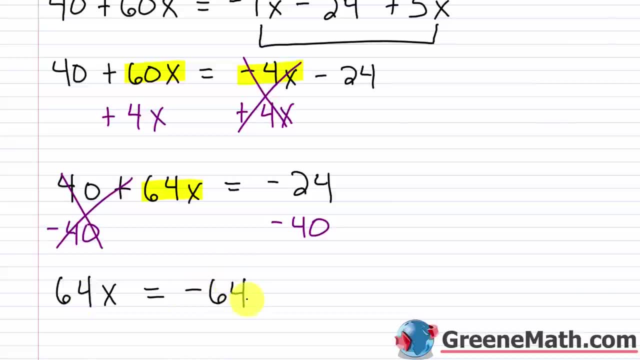 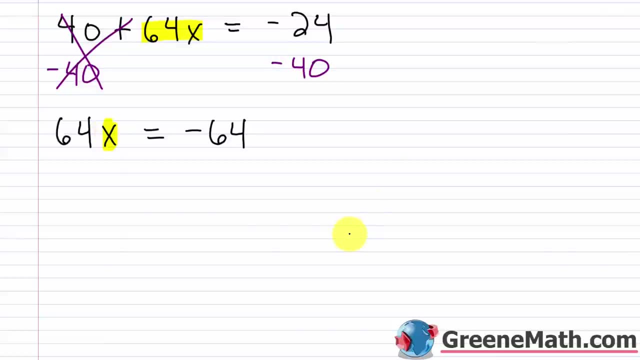 negative 24 minus 40 is negative 64. Now I just want my variable by itself. So I just want x. So how am I going to get that? Again, look at what's being done to x If we're multiplying. 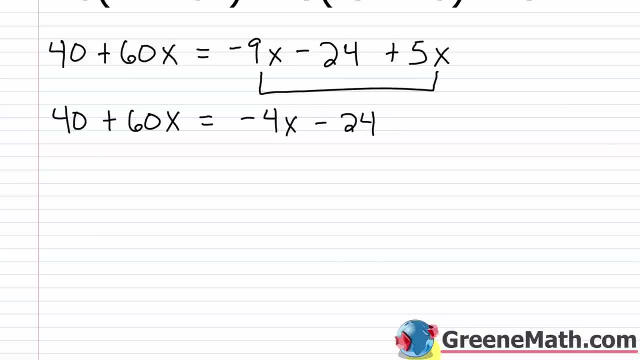 just a number on the other so in the previous examples it's been kind of easy to do that here what you're going to notice is that you have a variable term here and here now what you want to do is use the addition property of equality to get both on one side remember i can move anything so if i have negative 4x over here i can just add 4x and make it disappear on this side but i have to do the same thing over here to make it legal so in other words if i add 4x here it's going to disappear on this side negative 4x plus 4x 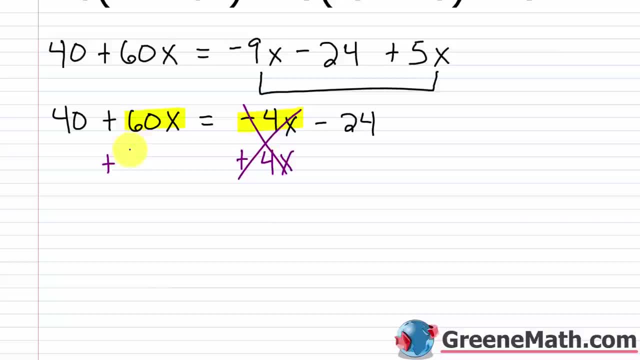 that's zero so it's gone but it reappears over here because i have to also do it on this side to make it legal so now i'll have 40 plus 60x plus 4x is 64x and this equals negative 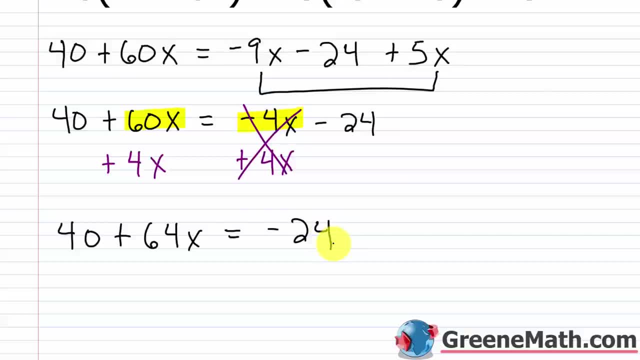 this is still not what i want because i want a variable term on one side of the equation 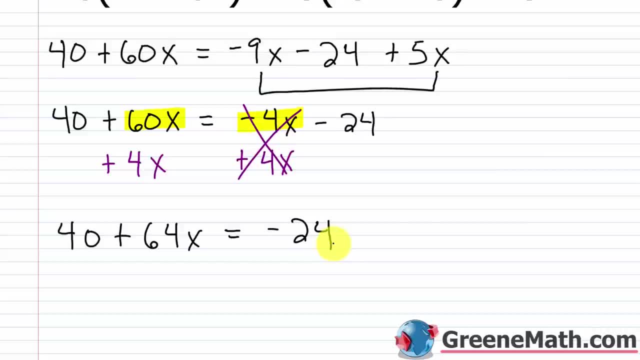 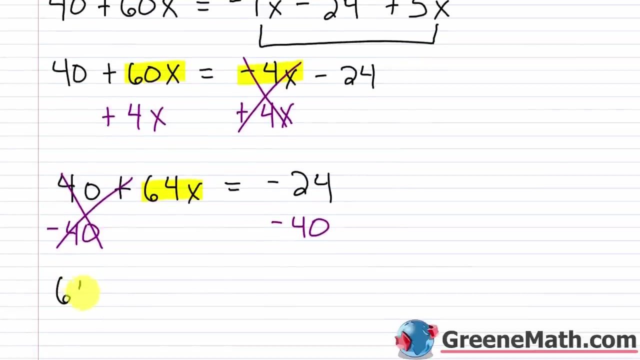 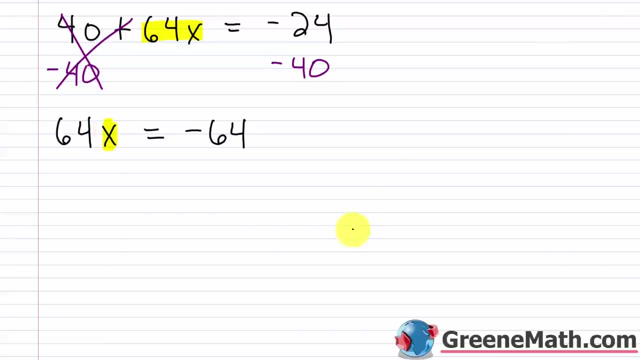 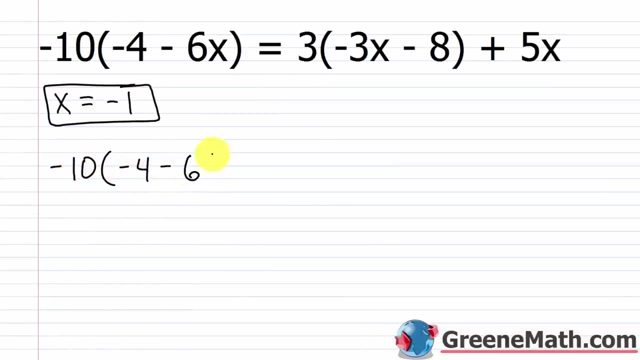 and i want just a number on the other so in order to do this again if i'm adding 40 to the variable term 64x to make this 40 go away i'm just going to subtract it away right but i have to do it to both sides that's the key so minus 40 over here and minus 40 over here so now this is gone and i have 64x on the left side so i've isolated the variable term on the right side negative 24 minus 40 is negative 64 now i just want my variable by itself so i just want x so how am i going to get that again look at what's being done to x if we're multiplying like we are here you have 64 that's multiplying x so you want to use division right to undo the multiplication so if i divide both sides of the equation by the coefficient of x i'm going to get 64x and i'm going to get 64x which is 64 i'm going to get x by itself this cancels with this remember 64 divided by 64 is 1 1 times x is just x over here negative 64 divided by 64 this gives me negative 1 so negative 1 x equals negative 1 is my solution all right so let's erase everything and check and so we'd have negative 10 times this quantity negative 4 minus 6 times negative 1 this equals 3 times this quantity negative 3 times negative 1 minus 8 then plus 5 times negative 1 and again all i'm doing is i'm plugging in a negative 1 ever everywhere that x exists so that means i 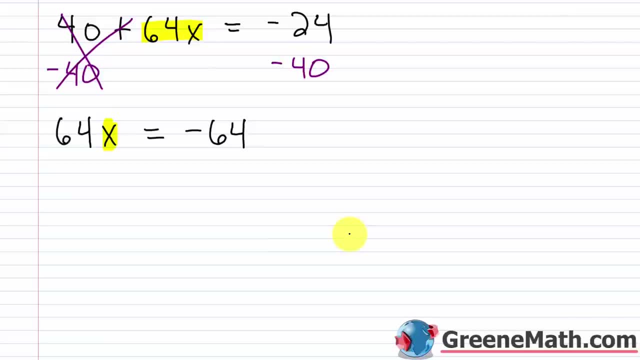 like we are here, you have 64, that's multiplying x. So you want to use division right To undo the multiplication. So if I divide both sides of the equation by the coefficient of x, which is 64, I'm going to get x by itself. 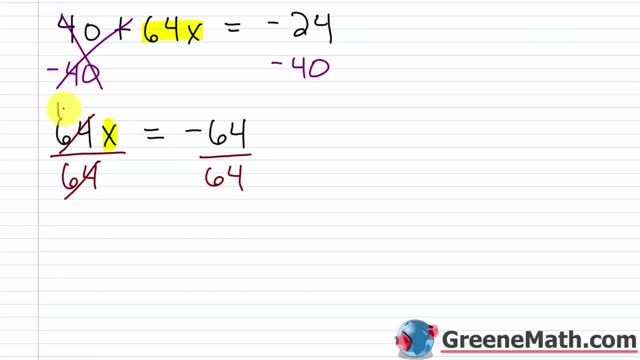 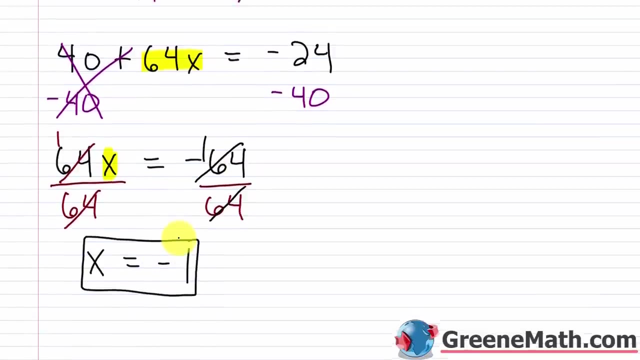 This cancels with this. Remember: 64 divided by 64 is 1.. 1 times x is just x Over here. negative 64 divided by 64, this gives me negative 1.. So negative 1, x equals negative 1 is my solution, All right, so let's erase everything and check. 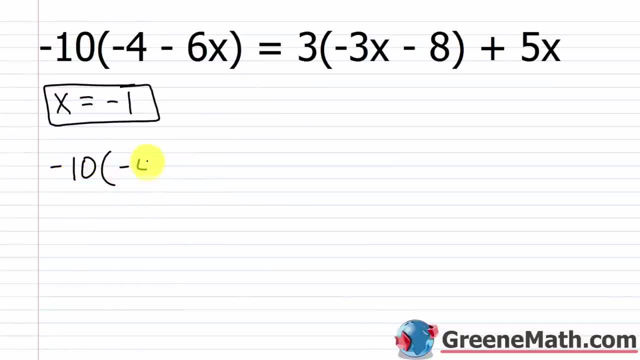 And so we'd have negative 10 times this quantity, negative 4 minus 6 times negative 1. This equals 3 times this quantity negative, 3 times negative, 1 minus 8, then plus 5 times negative 1.. And again, all I'm doing is I'm plugging in a negative 1 everywhere that x exists. 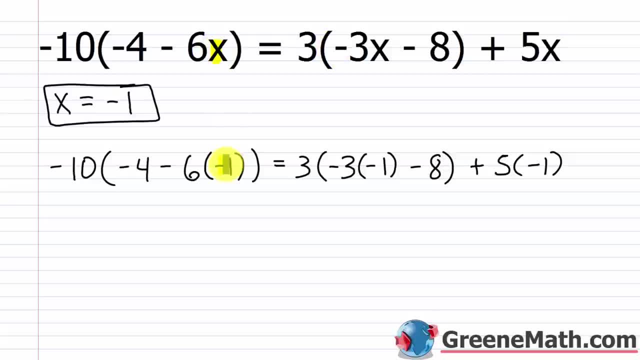 So that means I plugged in a negative 1 here, here and here And I'm just going to make sure the left and the right side are going to be the same value, right, Make sure they're equal. So on the left, I start inside the parentheses and I'm going to start with negative 6 times. 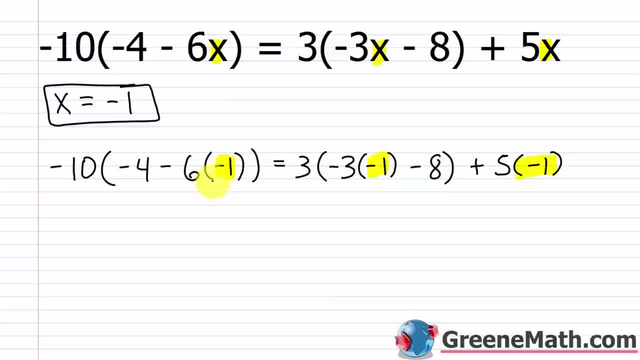 negative 1. That's 6. And so I'd have negative 4 plus 6. That's going to give me 2.. So this left side would be negative 10 times. 2. On the right side, inside the parentheses, negative 3 times. 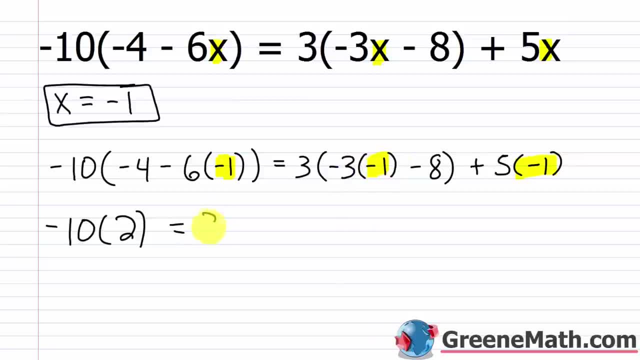 negative 1 is 3.. 3 minus 8 is negative 5.. So I'd have 3 times negative 5, and then plus 5 times negative 1.. Let's do all our multiplication: Negative 10 times 2 is negative 20.. 3 times: 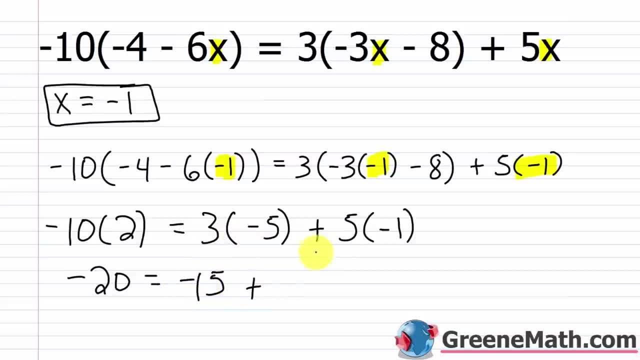 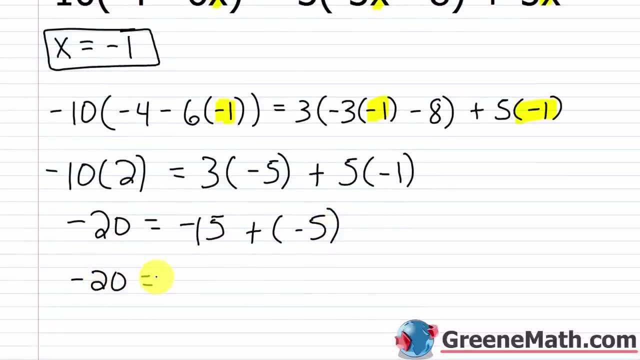 negative 5 is negative 15.. And plus 5 times negative 1 is negative 5.. You can kind of eyeball this and see how it works out. On the left, you have negative 20.. On the right, negative 15 plus. 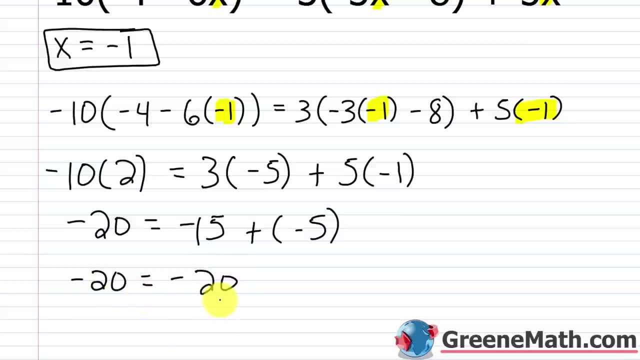 negative 5 is negative 20.. And so negative 20 equals negative 20.. We have the same value on each side of the equation, So we know that x equals negative 1 is the correct solution. Hello and welcome to another episode of the X-Equals-Negative-1.com. I'm your host. 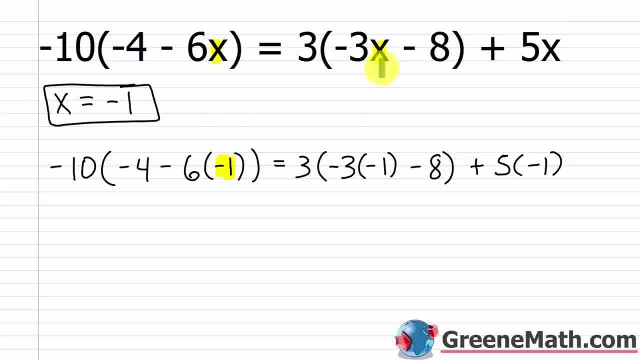 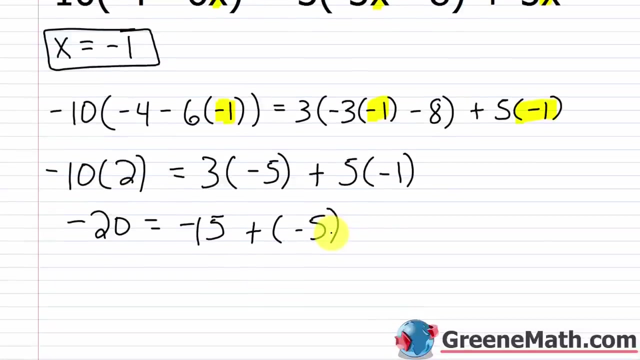 plugged in a negative 1 here here and here and i'm just going to make sure the left and the right side are going to be the same value right make sure they're equal so on the left i start inside the parentheses and i'm going to start with negative 6 times negative 1 that's 6 and so i'd have negative 4 plus 6 that's going to give me 2 so this left side would be negative 10 times 2 on the right side inside the parentheses negative 3 times negative 1 is 3 3 minus 8 is negative 5 so i'd have 3 times negative 5 and then plus 5 times negative 1 let's do all our multiplication negative 10 times 2 is negative 20 3 times negative 5 is negative 15 and plus 5 times negative 1 is negative 5 you can kind of eyeball this and see it works out on the left you have negative 20 on the right negative 15 plus negative 5 is negative 20 and so negative 20 equals negative 20 we have the same value on each side of the equation 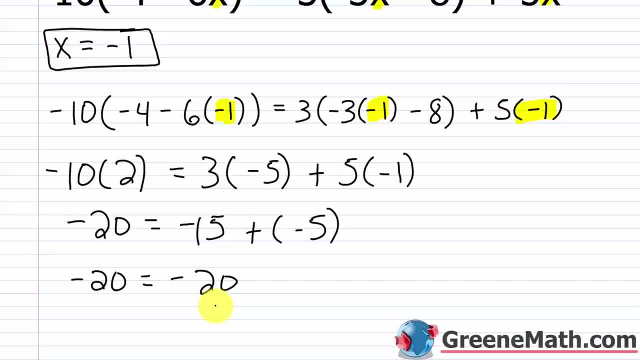 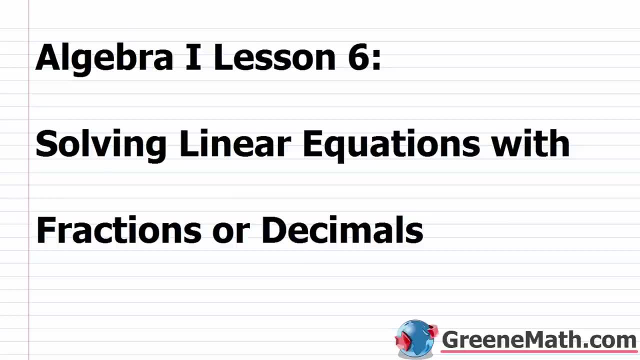 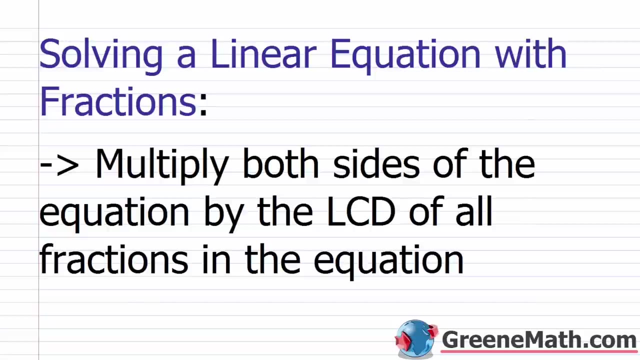 so we know that x equals negative 1 is the correct solution hello and welcome to algebra 1 lesson 6 in this video we're going to learn about solving linear equations with fractions or decimals so up to the point we really haven't worked a lot with equations that have fractions or decimals and i kind of did 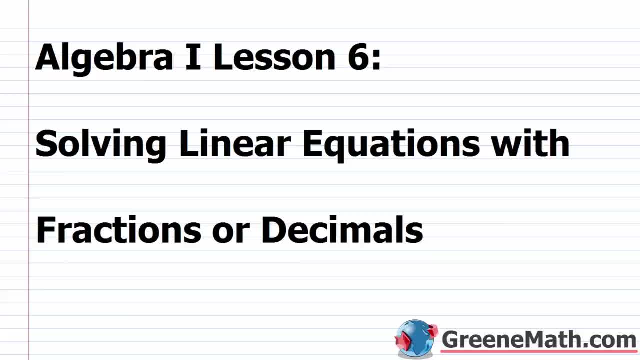 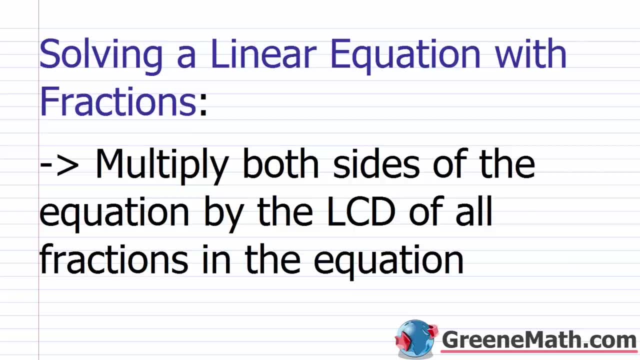 Algebra 1, Lesson 6.. In this video we're going to learn about solving linear equations with fractions or decimals. So up to this point we really haven't worked a lot with equations that have fractions or decimals, And I kind of did that to keep it very simple in the beginning. But 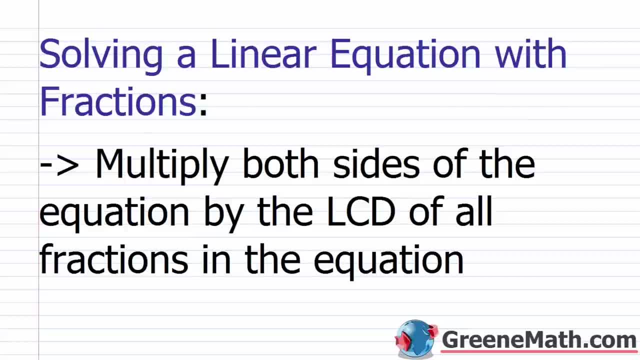 as you kind of progress through your chapter on solving linear equations in one variable, you're going to see a lot of problems with fractions and decimals. So when they occur we can use a special formula to solve them. So we're going to use a special formula to solve. 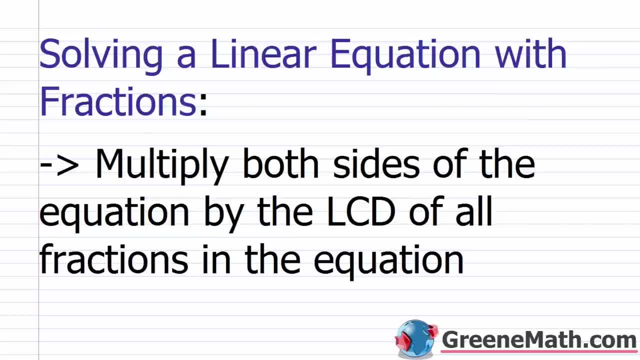 them. So let's first talk about how to solve a linear equation with fractions. Now, a lot of people hate fractions, So when they occur inside of an equation and you're just starting to learn equations, it makes it that much worse. right? You're already struggling to 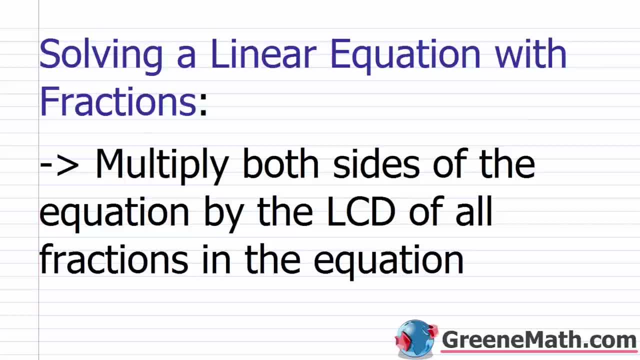 figure out how to solve an equation And now I'm throwing fractions in there And you're like, oh, what am I going to do? When you first start out the problem? you're going to clear your fractions by multiplying both sides of the equation by the LCD. Remember, that's called the. 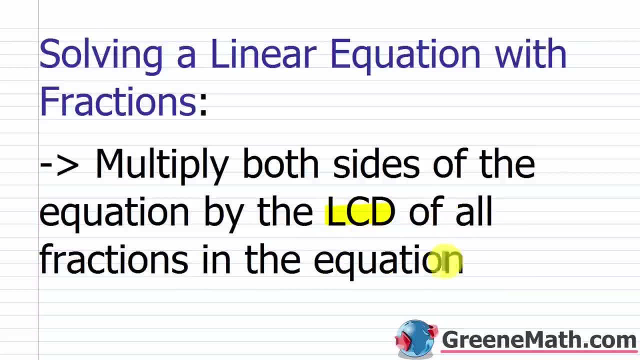 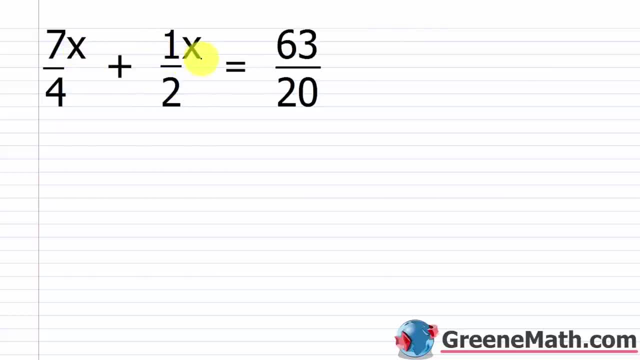 common denominator of all fractions in the equation. So, for example, we have seven fourths x plus one half x equals 63 over 20.. What you'll do is look at all your fractions. So here's a fraction. here's a fraction. here's a fraction. Okay, I want you to look at the denominators of. 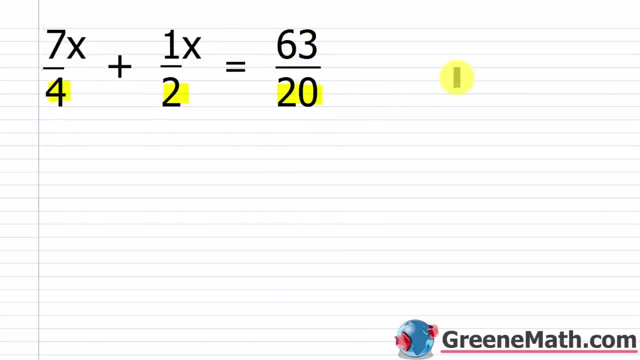 each fraction. So you have a four, you have a two and you have a 20.. So four, two and 20.. Those are my denominators. And we want the LCD. Remember the LCD is equal to the LCM. 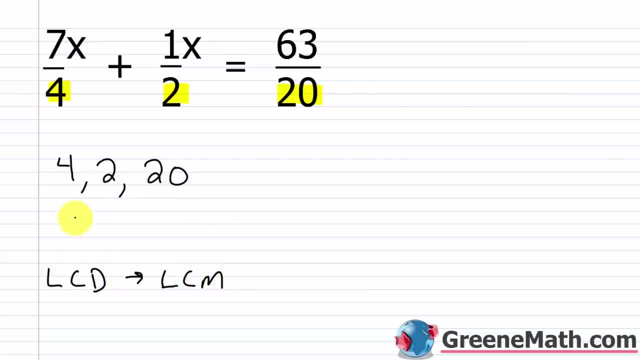 the least common multiple of the denominators. So what is the LCM of four, two and 20?? Well, remember from pre-algebra the way we figure this out: we would factor each number. So four would be four would be two times two. Two is a prime number that's not going to factor. 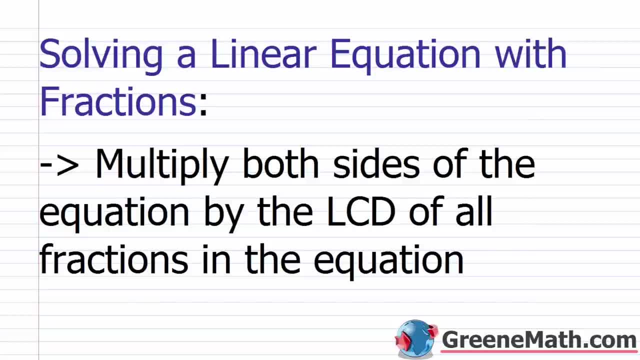 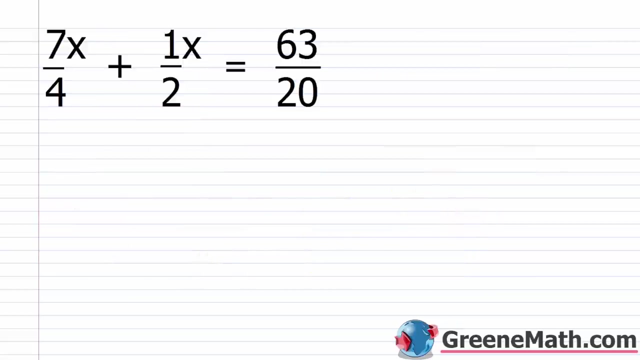 that to keep it very simple in the beginning but as you kind of progress through your chapter on solving linear equations in one variable you're going to see a lot of problems with fractions and decimals so when they occur we can use a special trick to get rid of them so let's first talk about how to solve a linear equation with fractions now a lot of people hate fractions so when they occur inside of an equation and you're just starting to learn equations it makes it that much worse right you're already struggling to figure out how to solve an equation and now i'm throwing fractions in there and you're like oh what am i going to do when you first start out the problem you're going to clear your fractions by multiplying both sides of the equation by the lcd remember that's called the least common denominator of all fractions in the equation so for example we have seven fractions and we're going to solve a linear equation with one force x plus one half x equals 63 over 20. what you'll do is look at all your fractions so here's a fraction here's a fraction here's a fraction okay i want you to look at the denominators of each fraction so you have a 4 you have a 2 and you have a 20 so 4 2 and 20 those are my denominators and we want the lcd remember the lcd is equal to the lcm the least common denominator least common multiple of the denominators so what is the lcm of 4 2 and 20. well remember from 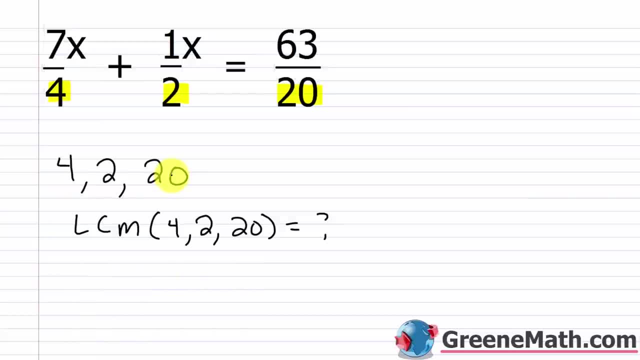 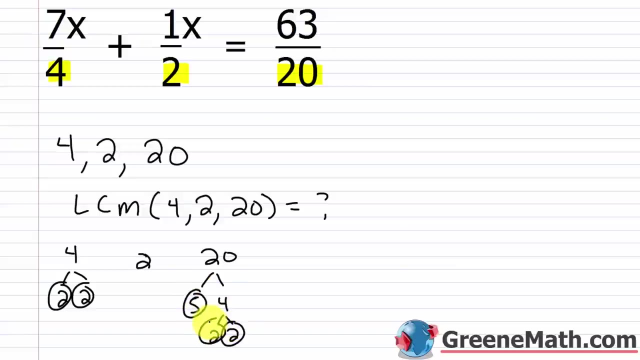 pre-algebra the way we figure this out we would factor each number so 4 would be 4 would be 2 times 2 2 is a prime number that's not going to factor and 20 is going to be 5 times 4 4 is 2 times 2 very very easy to do and to build the lcm we take each prime number from each prime factorization and we throw it in there the only thing is that you have to remember if a prime factor is repeated so in other words in 4 we have two factors of 2 in 2 we just have that number and in 20 we have two factors of 2 i put the largest number of repeats between all of the prime factors of 2 and the most recent prime factorizations so with the number 2 it occurs twice at most right it occurs twice here it occurs twice here so i'm going to put 2 in when i build my LCM and if that doesn't make any sense to you go back to the pre-algebra lesson on finding the least common multiple and it will make sense to you then alright now the next thing i want to put in here i have a 2 and a 2 i have a 2 here a 2 and a 2 here i only have a 5 left to put in so throw in a 5 and 2 times 2 is 4 times 5 is 20. So the LCM for 4, 2, and 20 is 20. So that means my least common denominator here is 20. Now, once I have figured that out, all I do is multiply both sides of the equation by that, and the fractions will go away. So I'll have 20 times 7 fourths x plus 1 half x 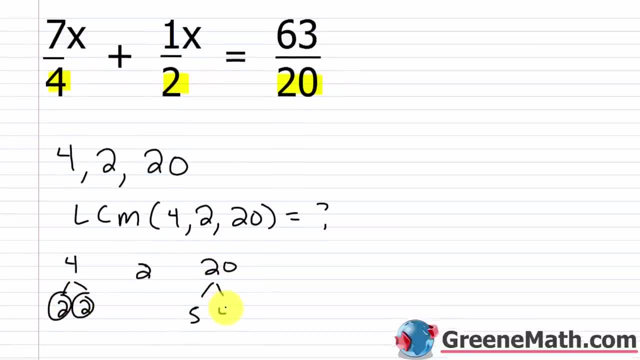 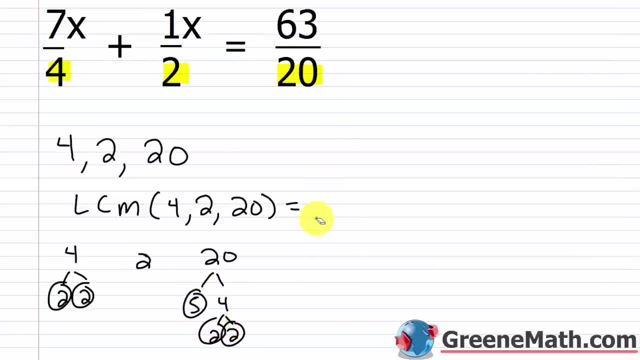 And 20 is going to be five times four. Four is two times two. Very, very easy to do And to build the LCM: we take each prime number from each prime factorization and we throw it in there. The only thing is that you have to remember if a prime factor is repeated. so in other words, in four. 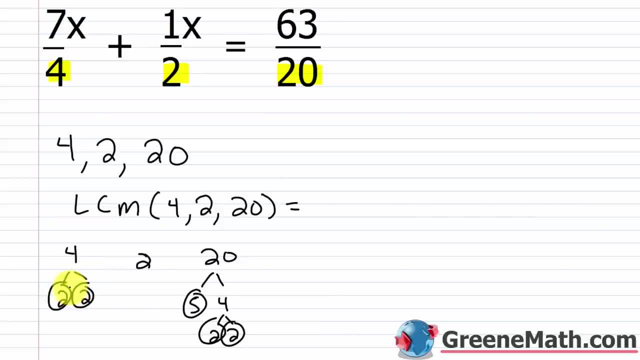 we have two factors of two. In 2, we just have that number, And in 20, we have two factors of 2.. I put the largest number of repeats between all of the prime factorizations. So with the number 2, it occurs twice at most, right. 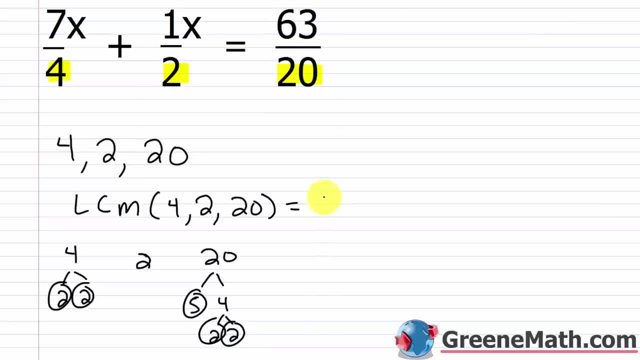 It occurs twice here. It occurs twice here, So I'm going to put 2 in when I build my LCM, And if that doesn't make any sense to you, go back to the pre-algebra lesson on finding the least common multiple, and it will make sense to you then. 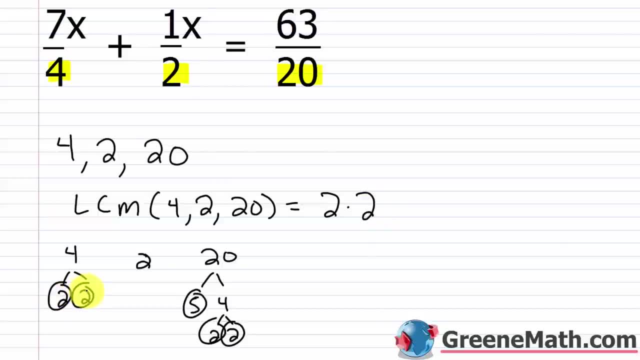 All, right. now the next thing I want to put in here. I have a 2 and a 2.. I have a 2 here, a 2 and a 2 here. I only have a 5 left to put in. 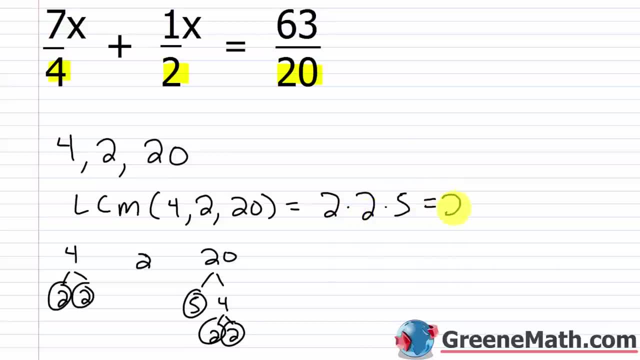 So throw in a 5, and 2 times 2 is 4.. 4 times 5 is 20.. So the LCM for 4,, 2, and 20 is 20.. So that means my least common denominator here is 20.. 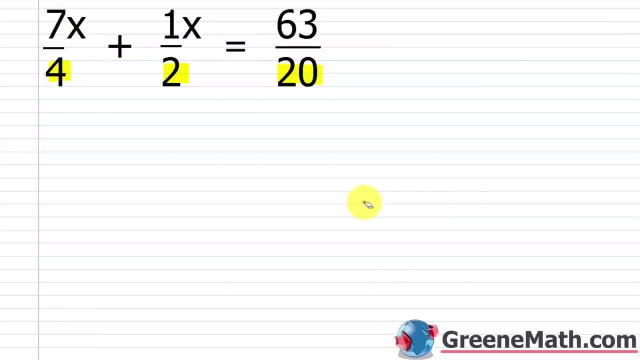 Now, once I have figured that out, all I do is multiply both sides of the equation by that and the fractions will go away, So I'll have 20.. Times 7 fourths x plus 1 half x equals 63 over 20 times 20.. 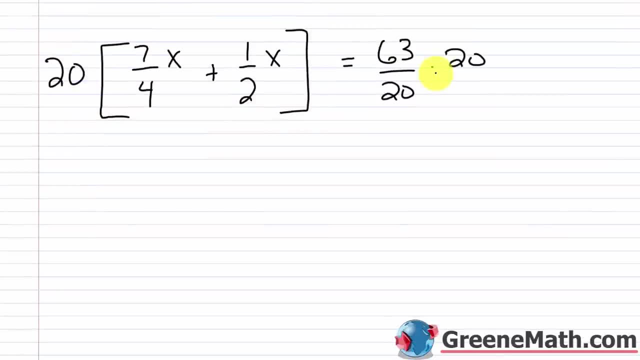 Now remember this is legal because of the multiplication property of equality. I can multiply both sides of an equation by the same non-zero number and preserve the solution. So on the right, it's pretty easy. This just cancels with this and I just get the number 63.. 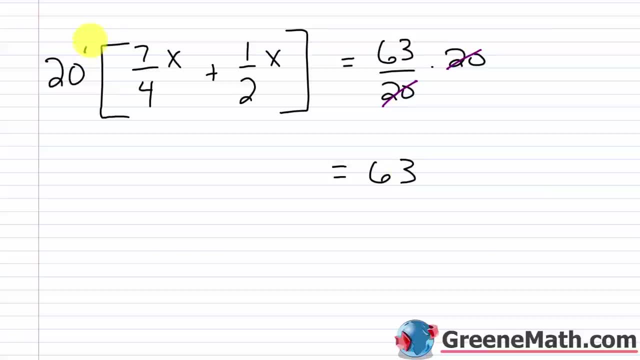 On the left, I've got to use my distributive property And I've got to distribute 20 to each term here. So I'm going to end up with 20 times 7 fourths x. So 20 times 7 fourths x, plus 20 times 1 half x. 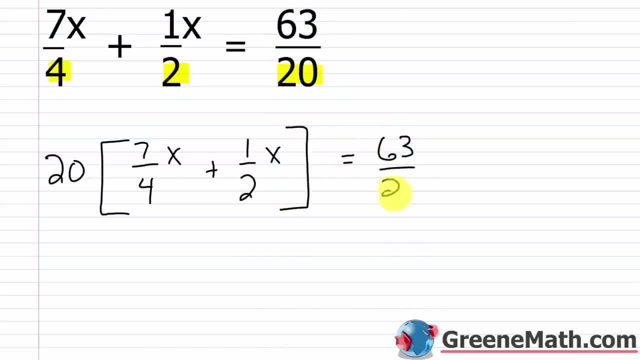 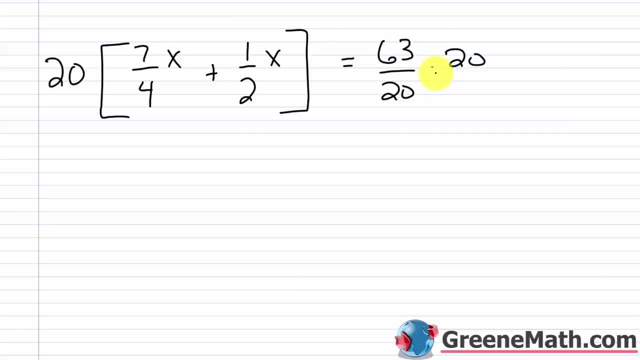 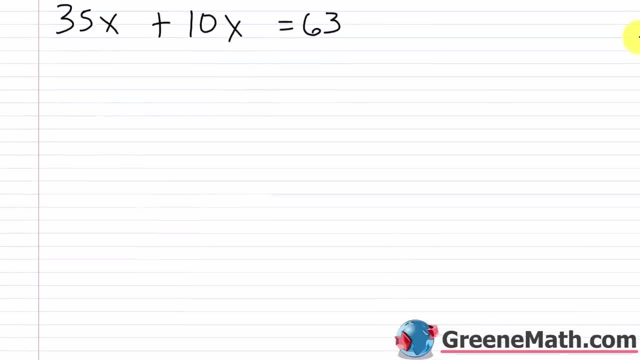 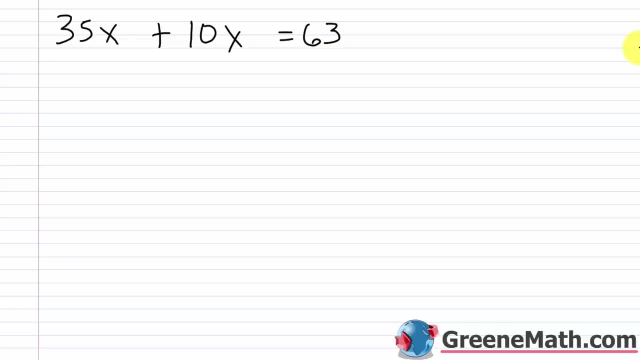 This equals 63, and we'll scroll down a little bit more. So now I have an equation that's clear of fractions, and the solution is going to be the same as if I had just worked with the fractions. 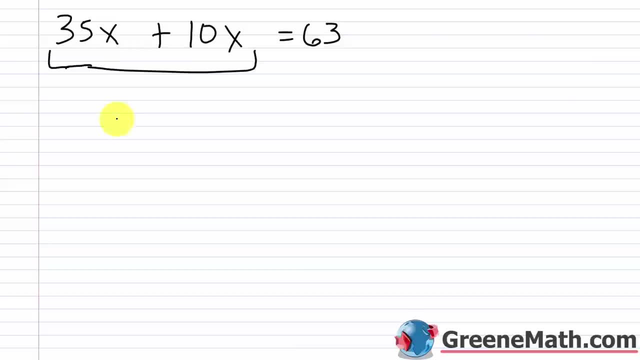 So I would start out by just combining like terms. 35x plus 10x is 45x, and this equals 63. 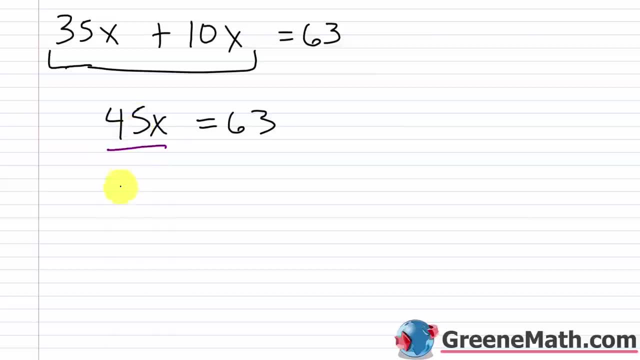 Now, to get x by itself, I divide both sides of the equation by the coefficient of x, which is 45. 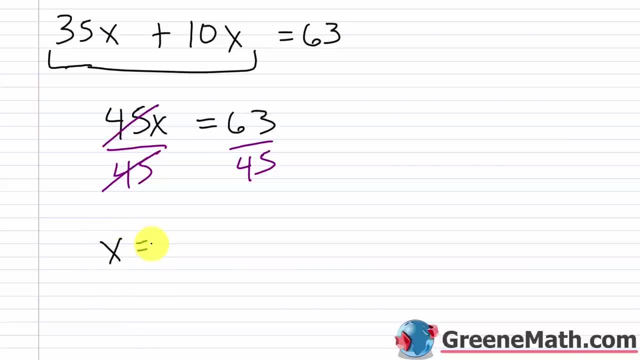 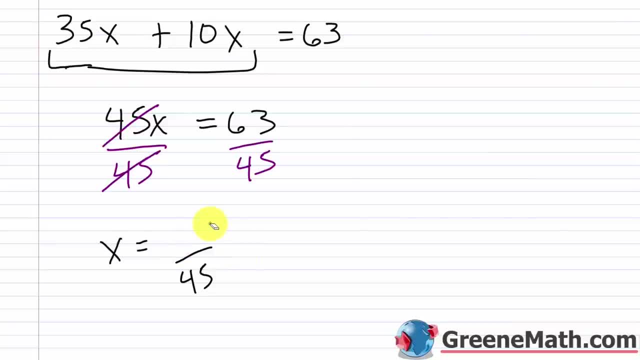 So I just have to reduce the fraction. So 63 is 9 times 7. 45 is 9 times 5. So the greatest common factor there is going to be 9. I can cancel this with 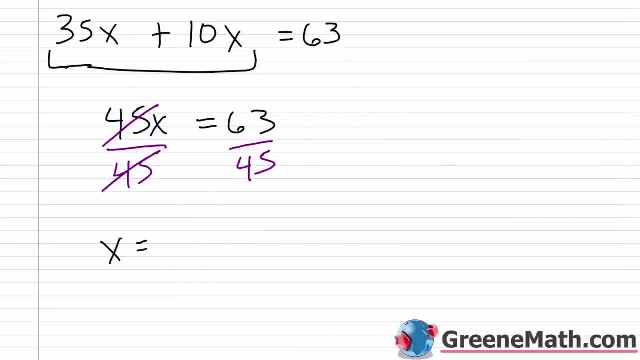 this, and I'll have 7 fifths, right? So x equals 7 fifths. 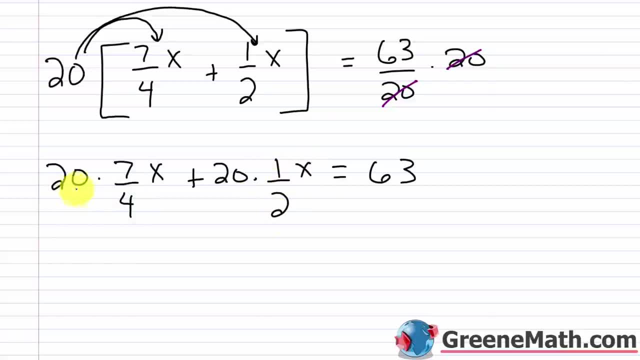 Now you can look and see: okay, between 20 and 7 fourths. this is going to cancel with this and give me 5.. 5 times 7 is 35, so I'm going to have 35x plus. 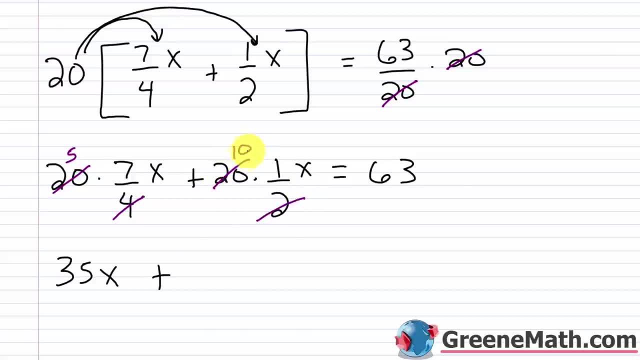 And then over here, This is going to cancel with this and give me a 10.. 10 times 1 is just still 10.. Then times x, so I'm going to have 10x there. This equals 63. And we'll scroll down a little bit more. 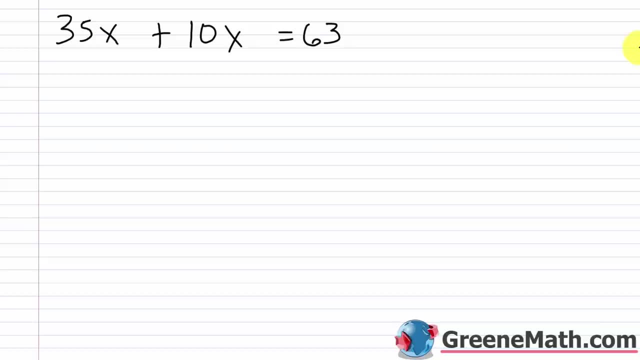 So now I have an equation that's clear of fractions And the solution is going to be the same as if I had just worked with the fractions. So I would start out by just combining like terms: 35x plus 10x is 45x. 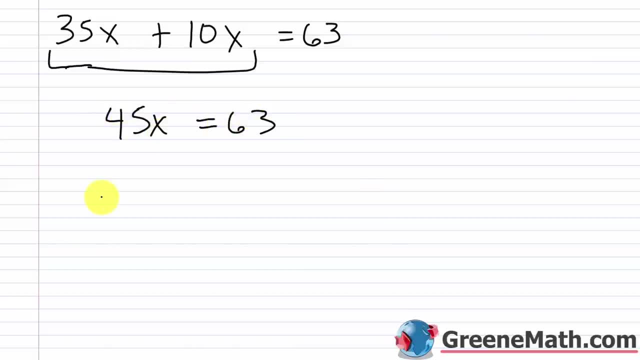 And this equals 63.. Now to get x by itself, I divide both sides, So I'm going to do the equation by the coefficient of x, which is 45. This will cancel with this and just give me an x And 63 over 45, that's not going to be a whole number. 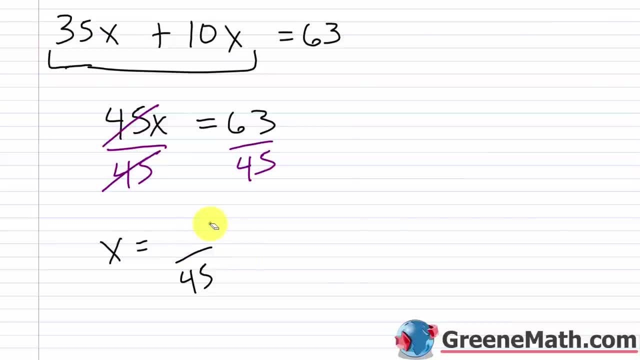 So I just have to reduce the fraction. So 63 is 9 times 7.. 45 is 9 times 5.. So the greatest common factor there is going to be 9.. I can cancel this with this And I'll have 7 fifths. 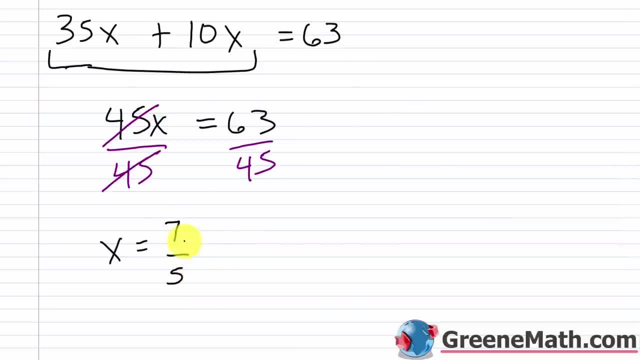 So x equals 7 fifths. You're going to get a lot of fractional solutions moving forward. I kind of stayed away from it in the beginning because I wanted to make everything nice and easy for you to understand before we start really ramping it up and dealing with fractions and decimals. 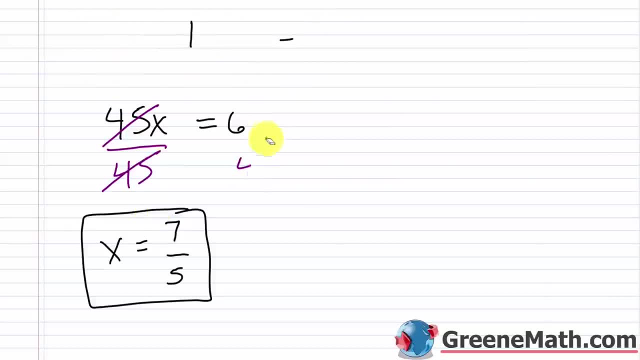 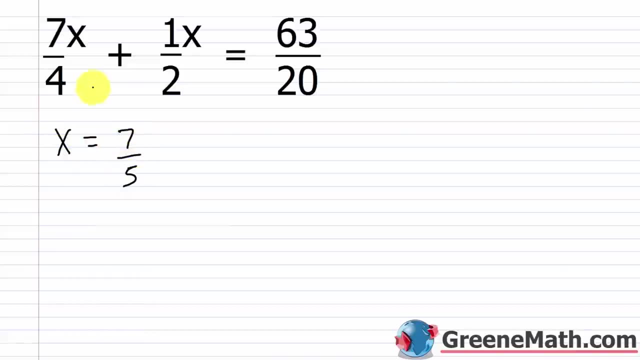 All right. so I want to do two things. I want to check this, So let's erase everything here, And we're going to go back up to the top. So remember: x equals 7 fifths, So I'm going to plug a 7 fifths in. 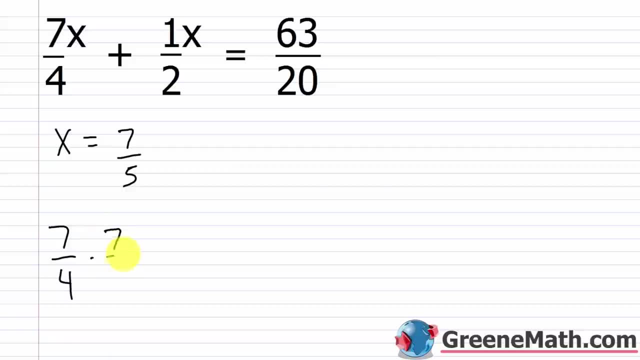 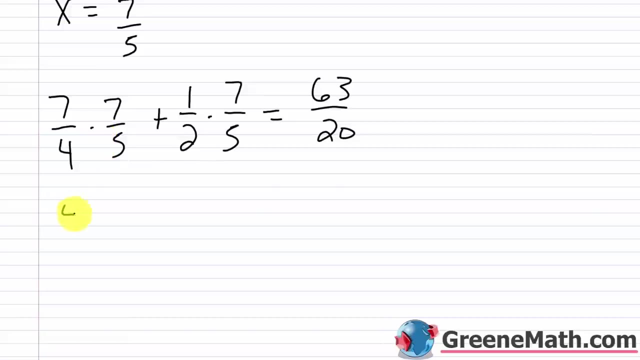 And everywhere I see an x. So 7 fourths times 7 fifths, plus 1 half times 7 fifths equals 63 over 20.. All right, So over here nothing I can cross cancel. So 7 times 7 is 49.. 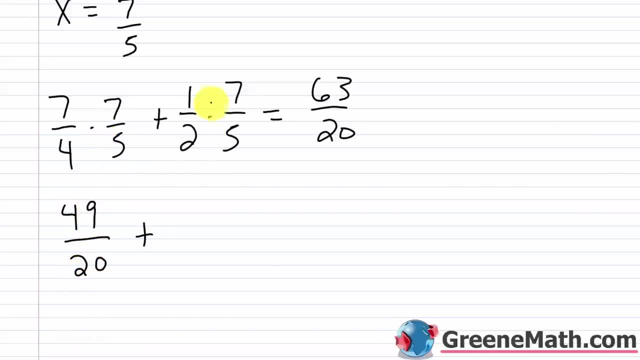 And 4 times 5 is 20.. Plus over here, nothing I can cross cancel. 1 times 7 is 7 over 2 times 5. That's 10.. Now, in order to add, I've got to have a common denominator. 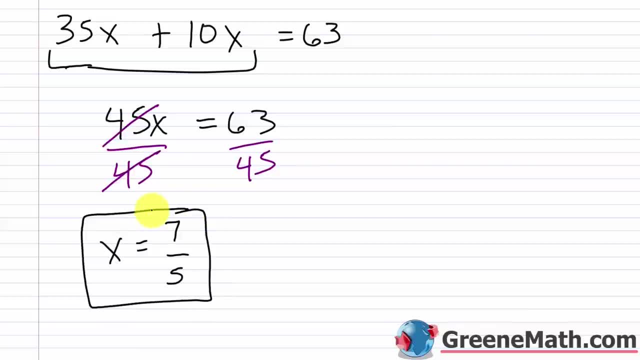 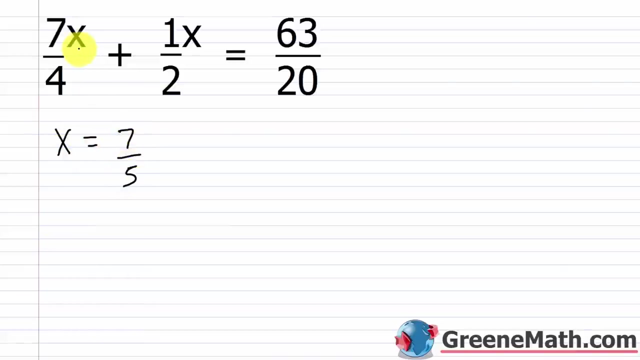 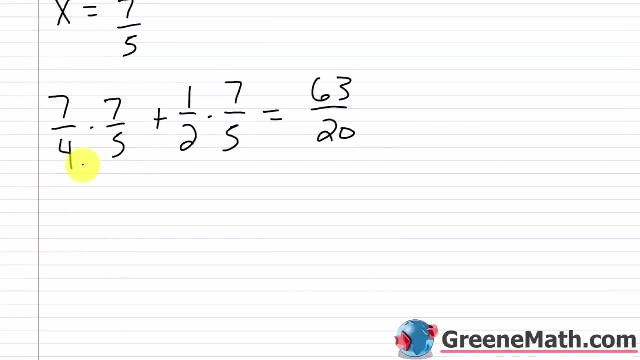 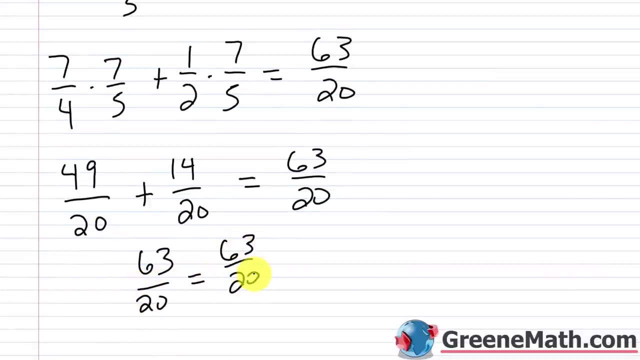 So I'm going to have 10 times 7. So I'm going to have 10 times 7. So I'm going to have 10 times 7. So I'm going to get a lot of fractional solutions moving forward. I kind of stayed away from it in the beginning because I wanted to make everything nice and easy for you to understand before we start really ramping it up and dealing with fractions and decimals. All right, so I want to do two things. I want to check this. So let's erase everything here. And we're going to go back up to the top. So remember, x equals 7 fifths. So I'm going to plug a 7 fifths in everywhere I see an x. So 7 fourths times 7 fifths plus 1 half. Times 7 fifths equals 63 over 20. All right. So over here, nothing I can cross cancel. So 7 times 7 is 49. And 4 times 5 is 20. Plus over here, nothing I can cross cancel. 1 times 7 is 7 over 2 times 5. That's 10. Now, in order to add, I've got to have a common denominator. So I'm going to go ahead and just multiply this by 2 over 2. And this will be 14 over 20. 14 over 20. And this equals 63 over 20. And of course, the left and the right side are going to be equal. 49 plus 14 is 63. This is over 20. And this is equal to 63 over 20. So our solution, x equals 7 fifths, is correct. One thing I want to show you, if we would have just left the fractions as is and just work with them, you're going to get the same answer. So clearing the 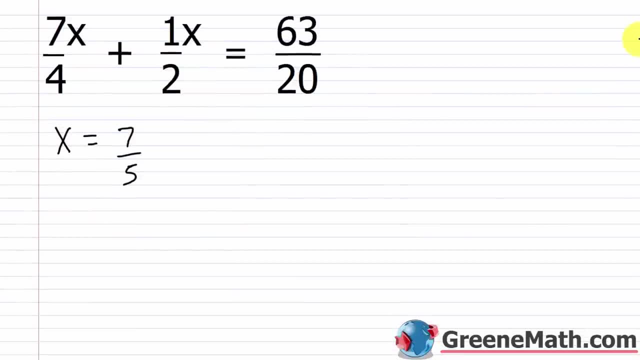 fractions is just more of a trick that you can use if you just don't like working with fractions. Sometimes it just makes it a lot easier, right? Nice and simple. So let's say I have 7 fourths. 7 fourths x plus 1 half x equals 63 over 20. If I want to, I can combine like terms here to simplify on the left. So move this kind of x over to the side 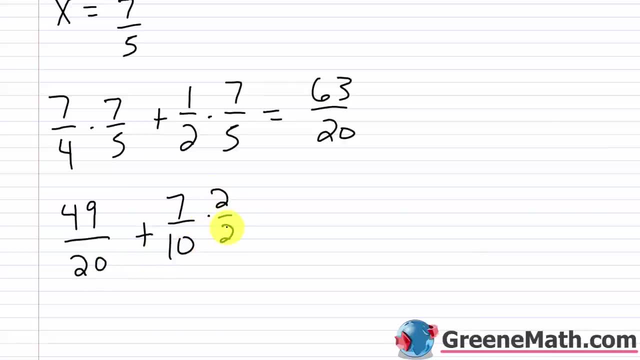 So I'm going to go ahead and just multiply this by 2 over 2. And this will be 14 over 20.. 14 over 20. And this equals 63 over 20.. And, of course, the left and the right side are going to be equal. 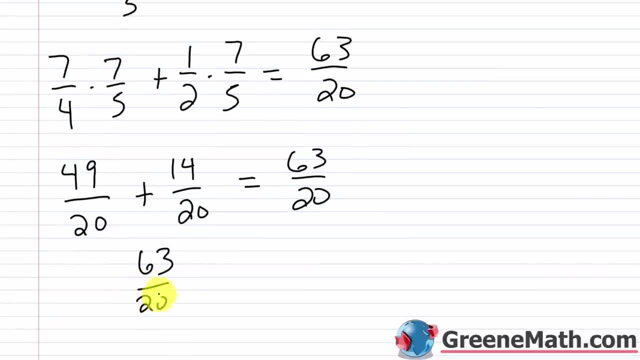 49 plus 14 is 63.. And this is over 20.. And this is equal to 63 over 20.. So our solution x equals 7 fifths is correct. One thing I want to show you. if we would have just left the fractions as is, 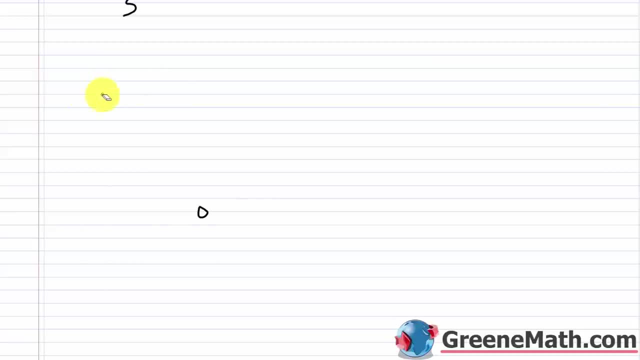 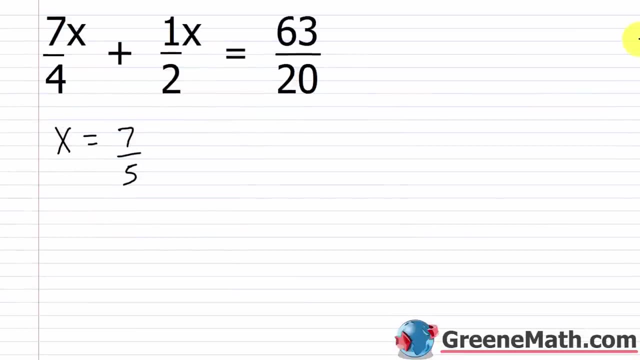 and just worked with them, you're going to get the same answer. So clearing the fractions- This is just more of a trick that you can use if you just don't like working with fractions. Sometimes it just makes it a lot easier. nice and simple. 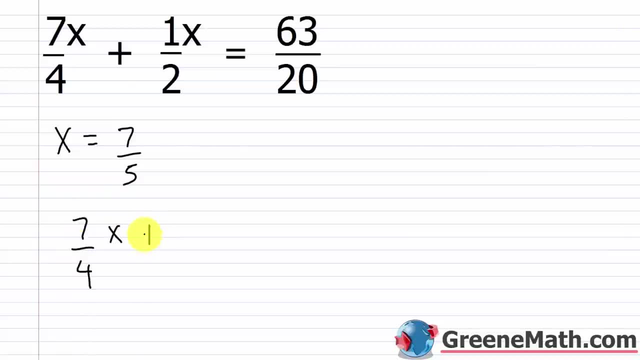 So let's say I have 7 fourths x plus 1 half x equals 63 over 20.. If I want to, I can combine like terms here to simplify on the left. So move this kind of x over to the side and get a common denominator. 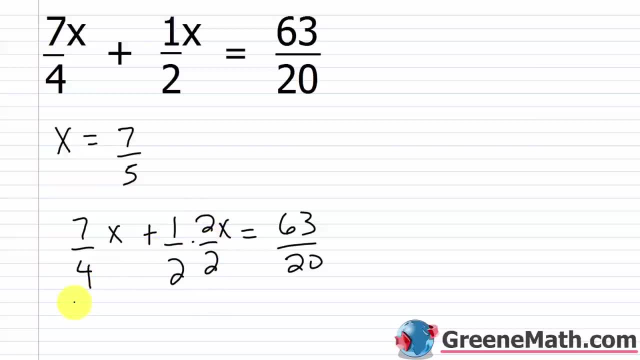 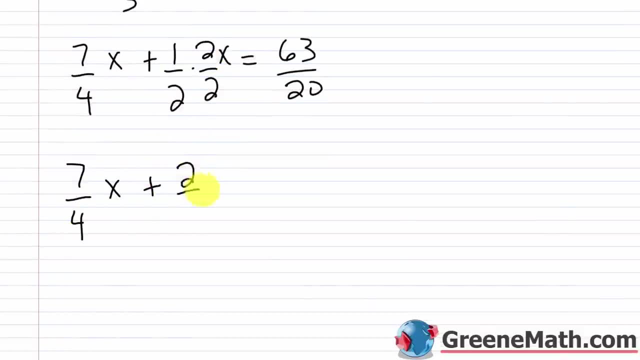 Multiply this by 2 over 2.. So then I'll have 7 fourths. Let me scroll down here. I'll have 7 fourths. x plus 1 times 2 is 2.. So 2 over 2 times 2 is 4.. 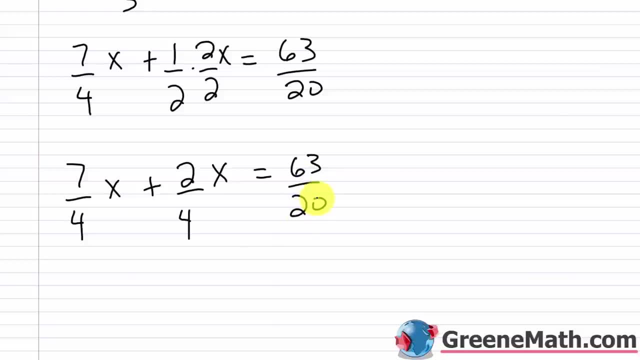 So 2 fourths x equals 63 over 20.. So to combine like terms here, I'm just going to add the numerator: 7 plus 2 is 9.. So I would have 9.. The common denominator is 4.. 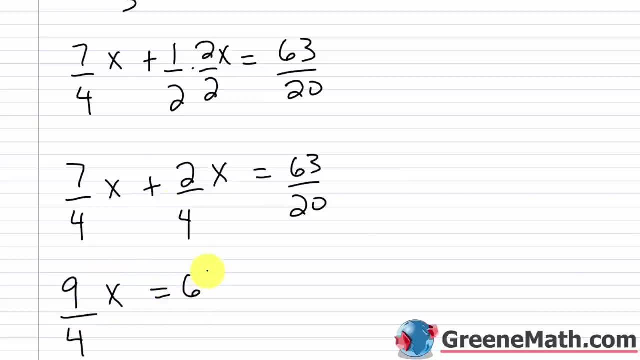 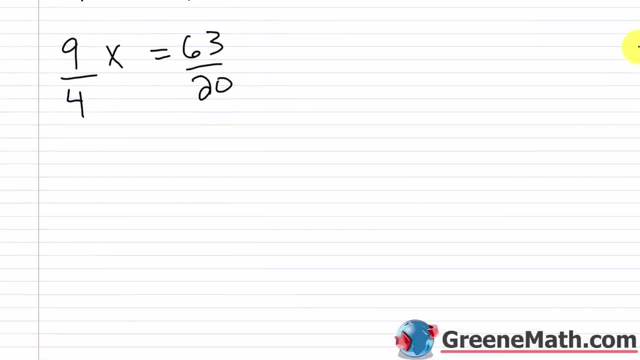 So 9 fourths then times x equals 63 over 20.. Now how do I isolate the variable here? We talked about it in one of our beginning video. We talked about the variable lessons. if I have a fractional coefficient for X and I want X by itself, 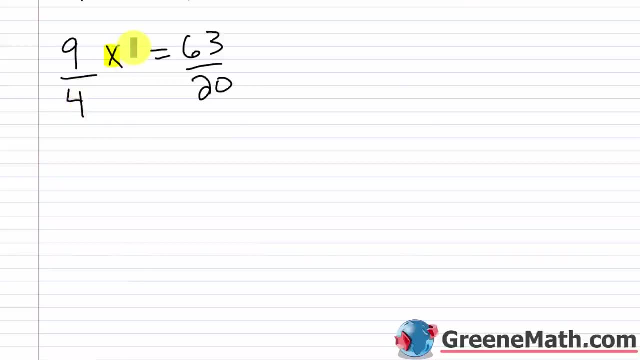 remember, if I multiply a number by its reciprocal, the result is 1. so if I multiply 9 fourths by 4 ninths, remember the reciprocal is found by taking the denominator and put it into the numerator. taking the numerator and put it into the denominator, I'm gonna get one right if I multiply these two. so 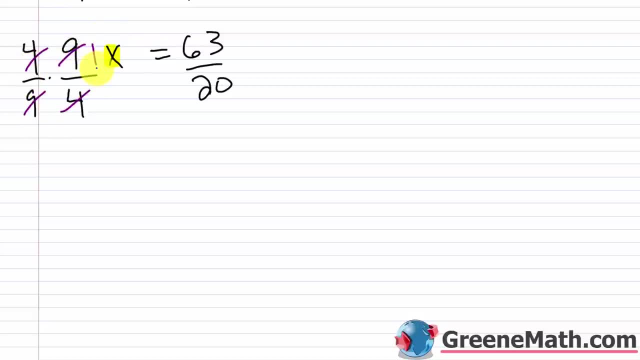 this, this, this, this, that all cancels. so this is 1x now, because I do it over here. I've got to do it over here. so this cancels with this and gives me 7, this cancels with this and gives me 5. so what am I gonna have? I'm gonna have X. 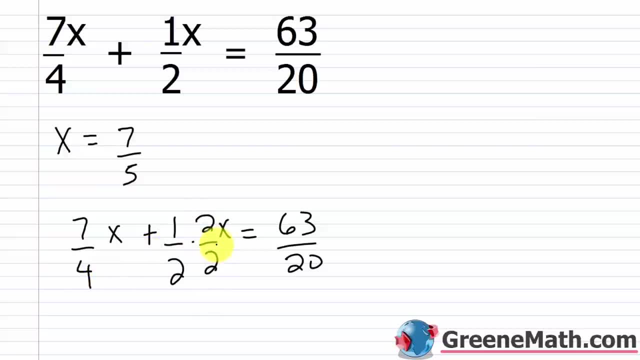 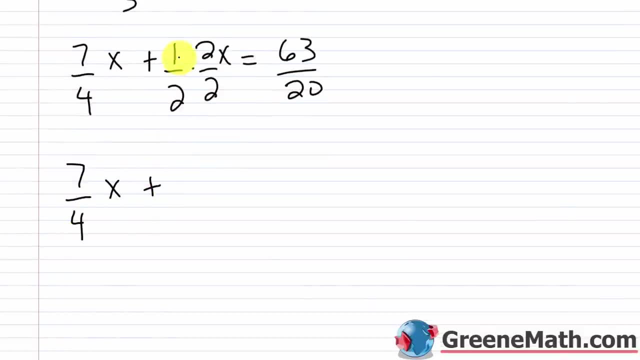 and get a common denominator. Multiply this by 2 over 2. So then I'll have 7 fourths. Let me scroll down here. I'll have 7 fourths x plus 1 times 2 is 2. So 2 over 2 times 2 is 4. So 2 fourths x equals 63 over 20. So to combine like terms here, I'm just going to add the numerator. 7 plus 2 is 9. So I would have 9. The common denominator is 4. So 9 fourths, then times x equals 63 over 20. Now, how do I isolate the variable here? We talked about in 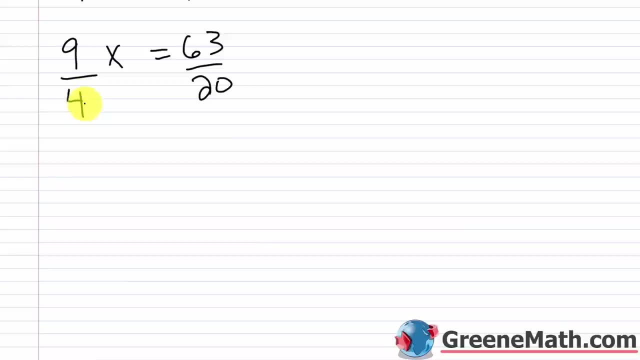 one of our beginning lessons, if I have a fractional coefficient for x and I want x by itself. Remember, if I multiply by x, I'm going to get x by itself. So I'm going to get x by itself. So if I multiply a number by its reciprocal, the result is 1. So if I multiply 9 fourths by 4 ninths, remember the reciprocal is found by taking the denominator and putting it into the numerator, taking the numerator and putting it into the denominator, I'm going to get 1, right, if I multiply these two. So this, this, this, this, that all cancels. So this is 1x. 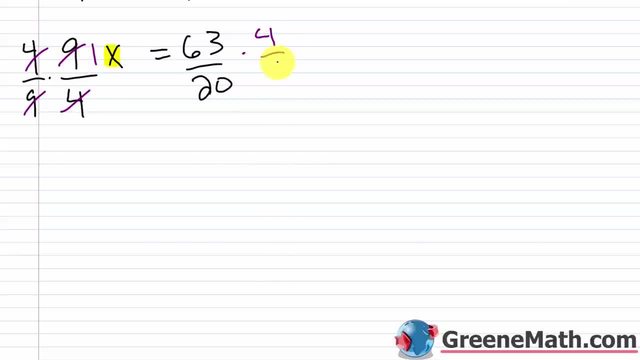 Now, because I do it over here, I've got to do it over here. So this cancels with this and gives me 7. This cancels with this and gives me 7. So this cancels with this and gives me 7. So this cancels with this and gives me 5. So what am I going to have? I'm going to have x equals 7 fifths. And 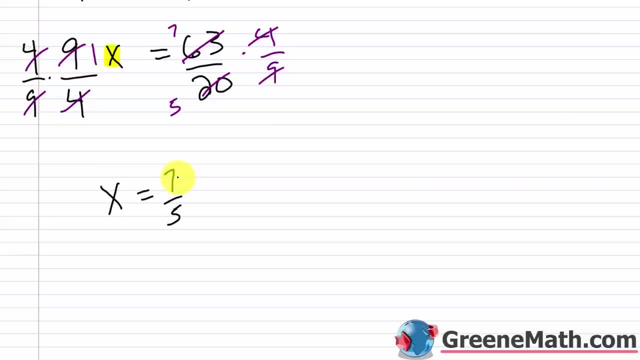 that's exactly what we got by clearing the fractions. Now, in this particular case, because I'm very good at working with fractions, right, I've been doing a long time, it didn't take me any longer to work this problem with the fractions involved. For yourself, you might not be that good 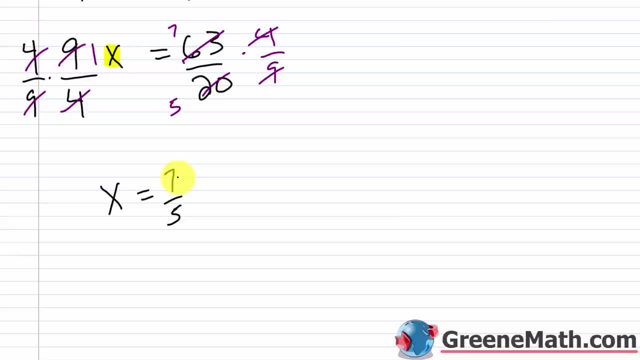 with fractions. So you might want to just take the time and clear the fractions so that you don't have the added stress of trying to solve an equation. 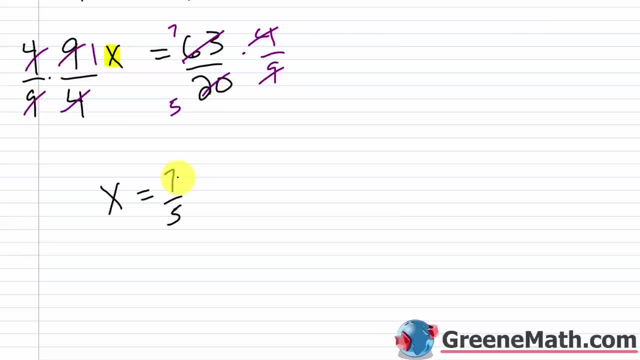 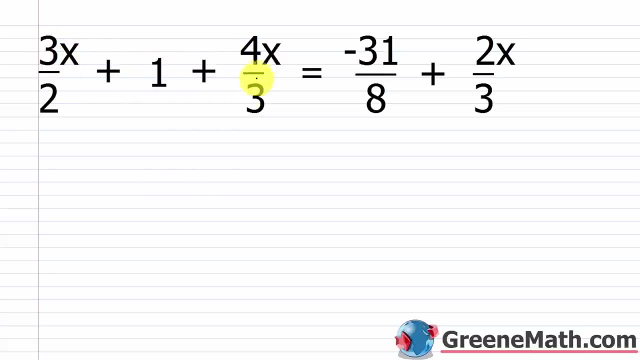 And trying to work with the fractions together. Now, when we get to decimals, because most of you work with calculators, you might not want to clear it. It might not save you any time. It just depends. All right, let's take a look at another one. So we have 3 halves x plus 1 plus 4 thirds x 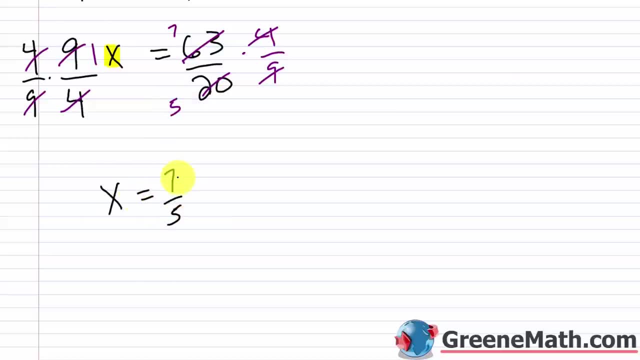 equals 7 fifths, and that's exactly what we got by clearing the fractions now in this particular case, because I'm very good at working with fractions, right- I've been doing a long time. it didn't take me any longer to work this problem with the 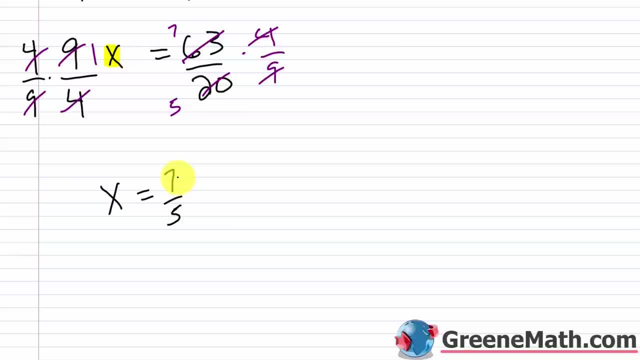 fractions involved for yourself. you might not be that good with fractions, so you might want to do that here, over here. I've got to do it over here. so this: to just take the time and clear the fraction so that you don't have the added stress of trying. 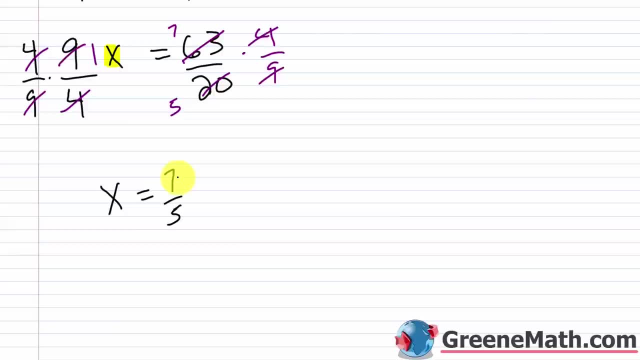 to solve an equation and trying to work with the fractions together. Now, when we get to decimals- because most of you work with calculators- you might not want to clear it. It might not save you any time, It just depends. All right, let's take a look at another one. So we have three. 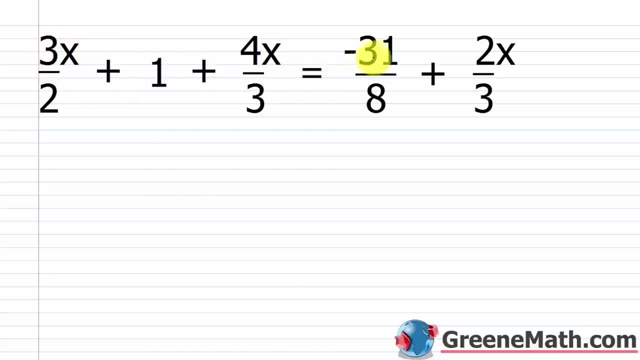 halves x plus one plus four thirds x equals negative 31 eighths plus two thirds x. All right, so what I'm going to do is again clear the fractions from the equation. So let's look at our denominators. We have a 2,, a 3,, an 8, and a 3.. Now I'm looking for the LCD, the least common. 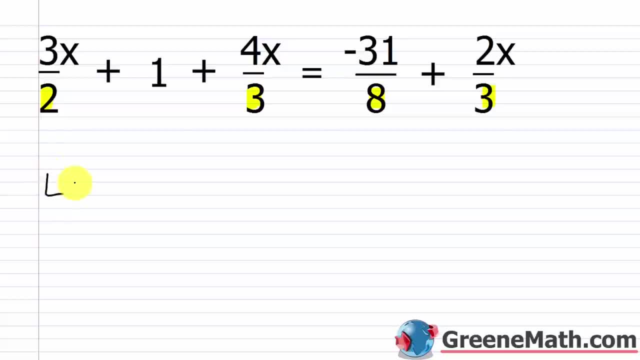 denominator And the way I find that I want the least common multiple of the denominator So 2,, 3, and 8.. And I'm not going to use the least common multiple of the denominator So 2,, 3, and 8.. 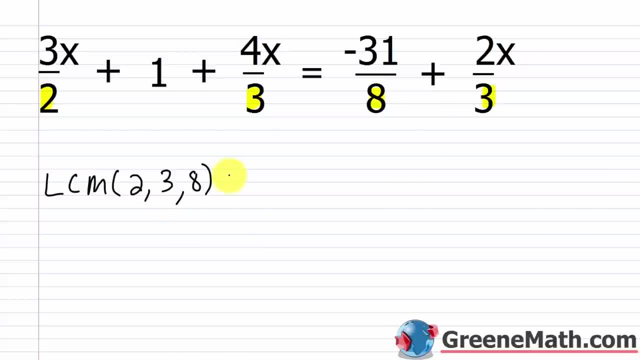 And I'm not going to use the least common multiple of the denominator, So 2,, 3, and 8.. going to put three in twice. right, it's the same number. so two doesn't factor, so i'm just going to throw that in there. three doesn't factor, just going to throw that in there. and eight is three. 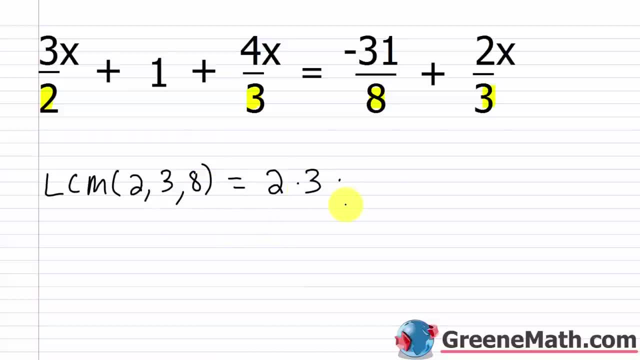 factors of two. so how many factors of two am i going to put in when i'm building my lcm? only three, right? so i'm going to put one and then two, because i already have one over here from when i did this. remember, when you build your lcm, you want the largest number of repeats between any of the 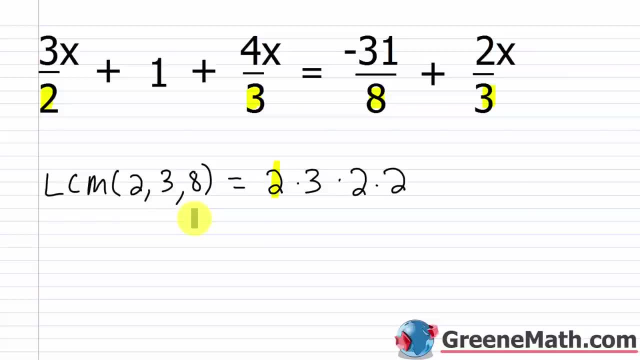 prime factorizations. so between eight you have one, two, three and two you have one. the largest number of repeats is three, so three goes in when you build this. okay, so we have two times three, which is six times two, which is 12 times two, again, which is 24. so that's going to be my lcm. 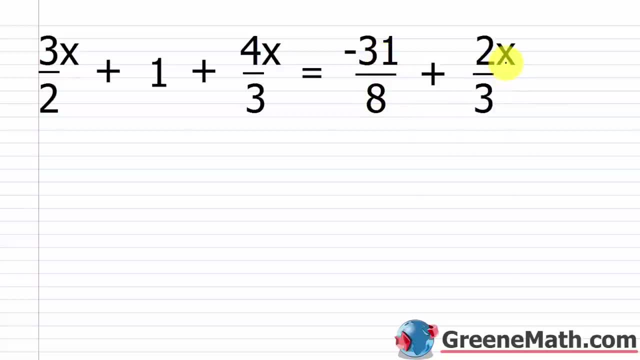 equals negative 31 eighths plus 2 thirds x. All right, so what I'm going to do is, again, clear the fractions from the equation. So let's look at our denominators. We have a 2, a 3, an 8, and a 3. Now, I'm looking for the LCD, the least common denominator. And the way I find that, I want the least common multiple of the denominators. So 2, 3, and 8. And I'm not going 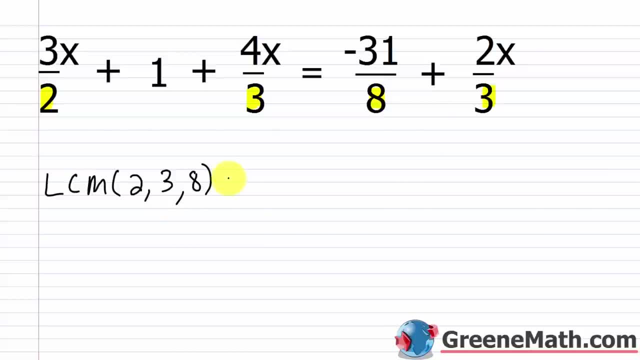 to put 3 in twice, right? It's the same number. So 2 doesn't factor. So I'm just going to throw 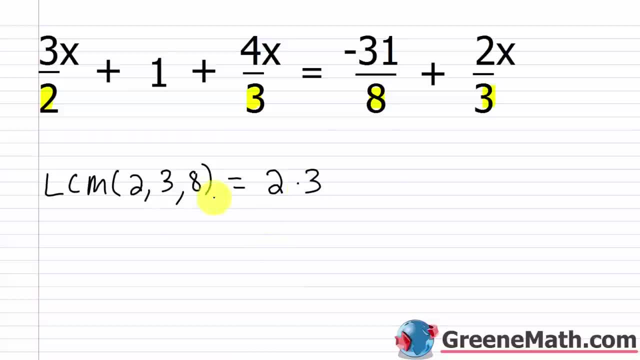 that in there. 3 doesn't factor. I'm just going to throw that in there. And 8 is 3 factors of 2. So how many factors of 2? 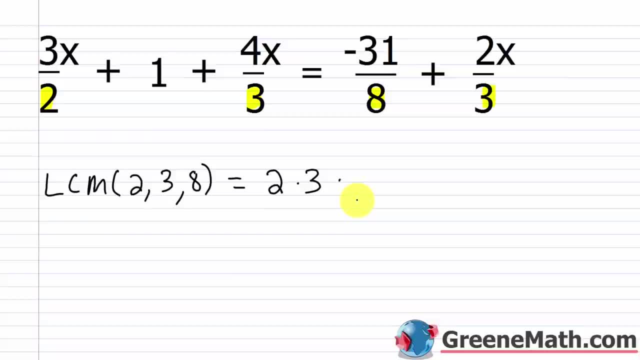 Am I going to put in when I'm building my LCM? Only 3, right? So I'm going to put 1 and then 2 because I already have 1 over here from when I did this. Remember, when you build your LCM, you want the largest number of repeats between any of the prime factorizations. So between 8, you have 1, 2, 3. And 2, you have 1. The largest number of repeats is 3. So 3 goes in when you build this. Okay, so we have 2 times 3, which is 6, times 2, which is 3. So we have 2 times 3, which is 2, which is 12, times 2 again, which is 24. So that's going to be my LCM for those numbers. 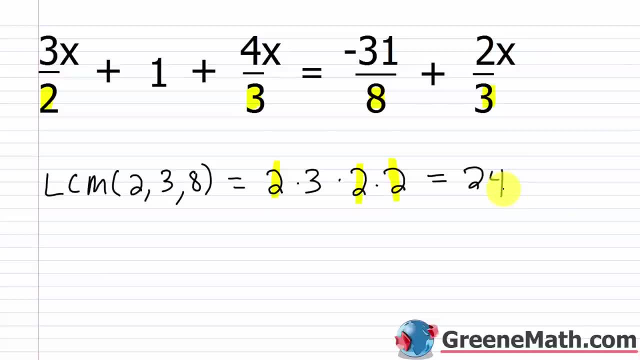 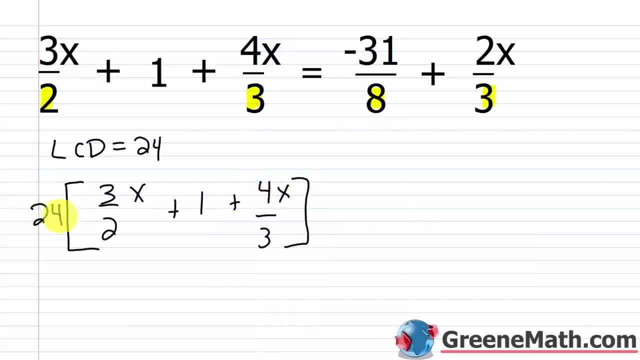 okay, you need to distribute this value of 24 to each term. i see a lot of students will just write 24 next to this and then they multiply by that and then they're done. that's. you need to multiply 24 by every term to make this legal. okay, so over here, negative 31 eighths plus two-thirds x, and we'll enclose this. 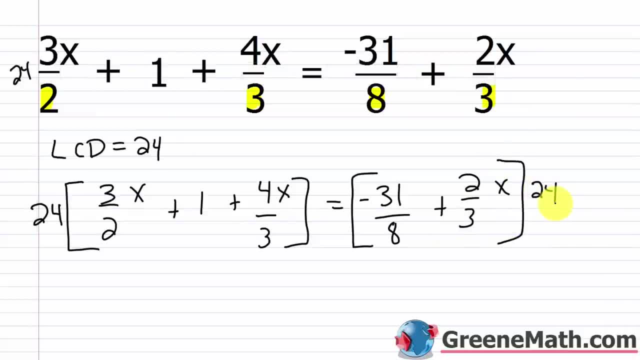 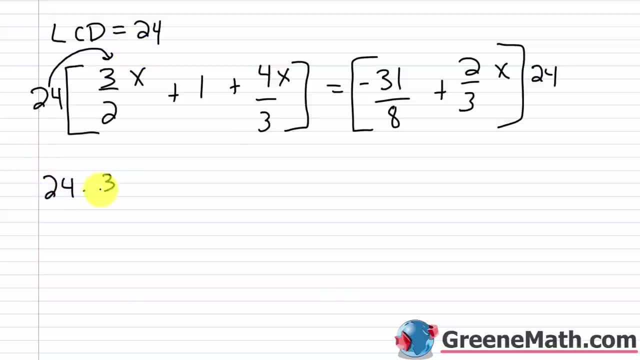 inside some brackets as well, and then we'll use our distributive property. so what i'm going to do, i'm going to multiply 24 by three-halves x, so 24 times three-halves x. and as i do it, i'm just going. 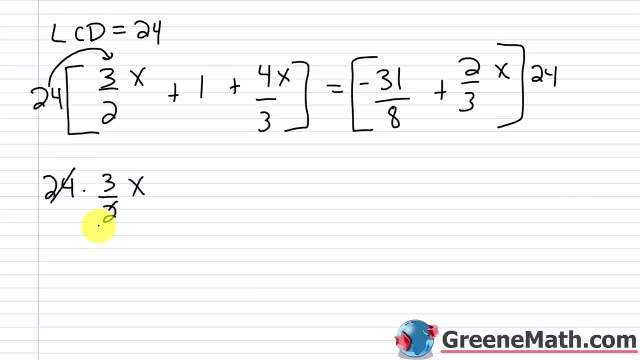 to do the calculation, kind of save some time. so 24 would cancel with 2 and give me 12. 12 times 3 is 36, so this would be 36, and then i'm going to multiply 24 by three-halves x and then i'm going to multiply. 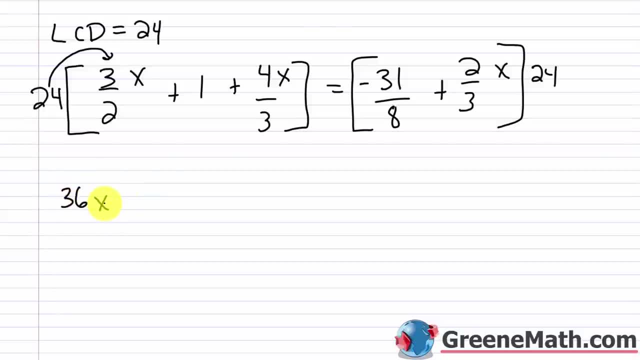 36 x. this is 36 x, okay, plus next i'd have 24 times 1. that's very simple, that's just 24. then plus next i'd have 24 times four-thirds x. so 24 times four-thirds x, the 24 would cancel. 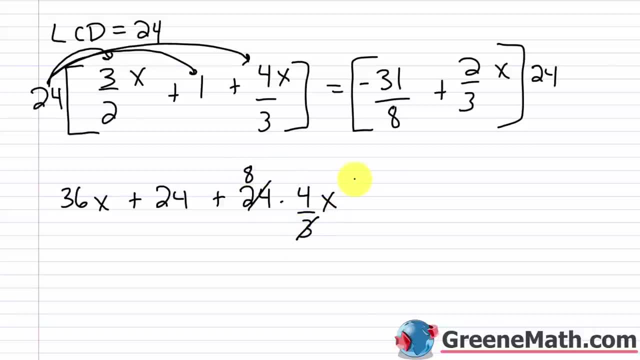 with the 3 and give me an 8. 8 times 4 is 32, so this would be 32 x 32 x, and then this equals- i'm going to do the same thing over here. so 24 times negative 31 eighths. so negative 31 eighths. 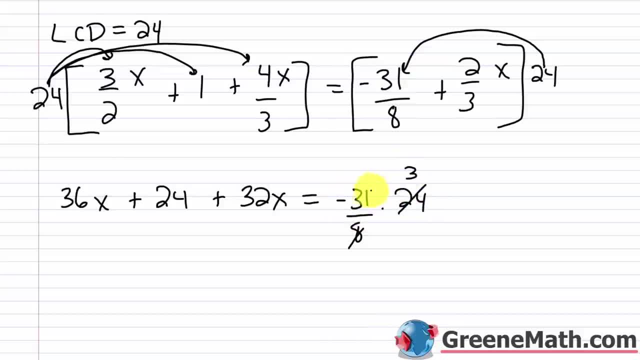 times 24. this cancels with this and gives me a 3, 3 times negative. 31 is negative 93, so negative 93. and then i have one more 24 times two-thirds x, so that's going to be plus two-thirds x times 24. and this 24, we cancel with this 3 and give me an 8. 8 times 2x is 16x. so this: 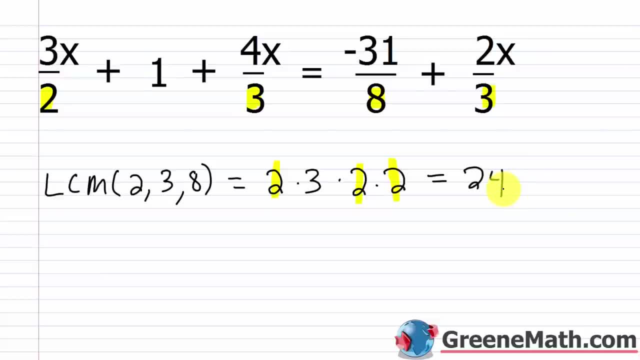 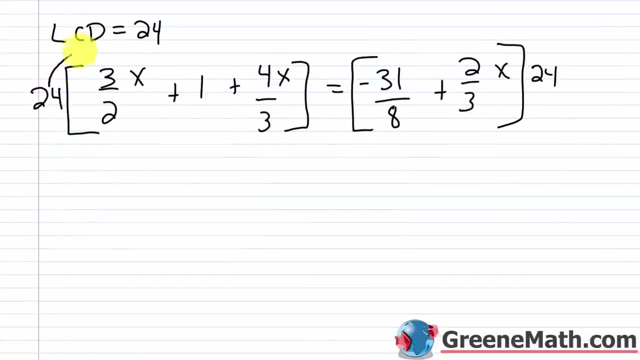 And so my least common denominator is 24. All right. So LCD is equal to 24. And so I multiply 24 by both sides of the equation. So I'm going to put some brackets here. Very important that you use brackets or parentheses because you need to distribute okay, you need to distribute this value of 24 to each term. I see a lot of students will just write 24 next to this. And then they multiply by that and then they're done. That's you need to multiply 24 by every term to make this legal. Okay, so over here, negative 31 eighths plus two thirds x. And we'll enclose this inside some brackets as well. And then we'll use our distributive property. So what I'm going to do, I'm going to multiply 24. By three halves x. So 24 times three halves x. And as I do it, I'm just going to do the calculation kind of save some time. So 24 would cancel with two and give me 12. 12 times three is 36. 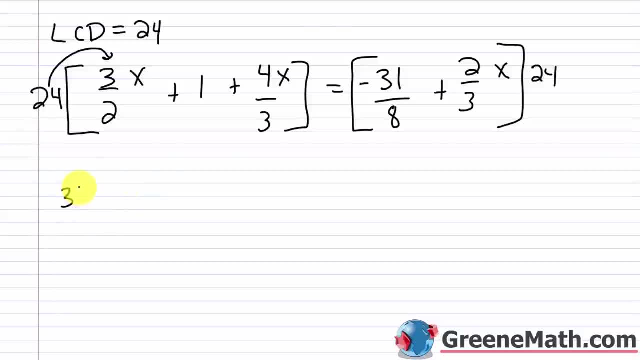 So this would be 36x. This is 36x. Okay, plus. Next, I'd have 24 times one. That's very simple. That's just 24. Then plus. Next, I'd have 24 times four thirds x. So 24 times, four thirds x. The 24 would cancel with the three and give me an eight. Eight times four is 32. 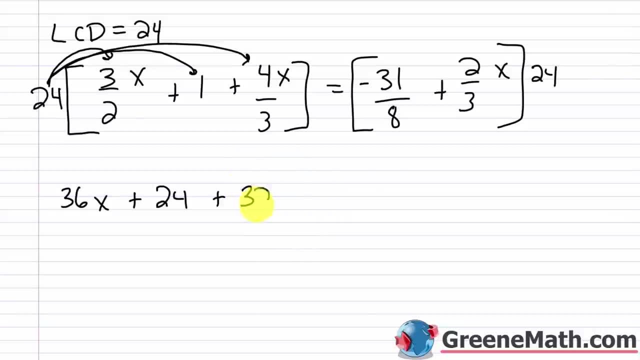 So this would be 32x. 32x. And then this equals, I'm going to do the same thing over here. So 24 times negative 31 eighths. So negative 31 eighths times 24. This cancels with this and 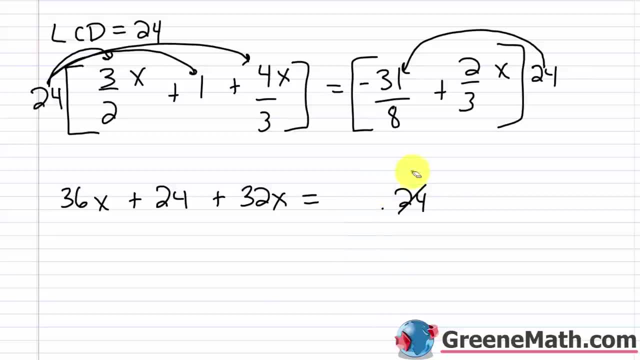 gives me a three. Three times negative 31 is negative 93. So negative 93. 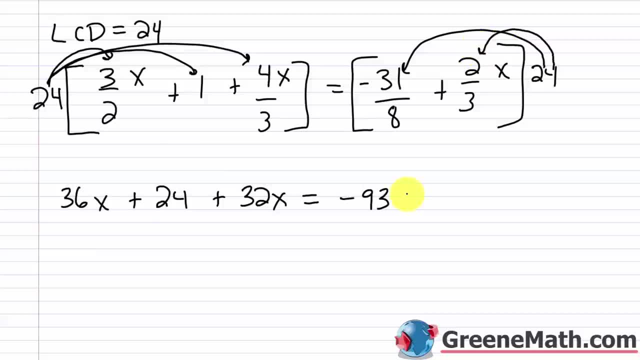 And then I have one more. 24 times two thirds x. So that's going to be plus two thirds x times 24. And this 24 would cancel with this three and give me an eight. Eight times two x is 16x. So this would be 16x. Okay, so now we're free of fractions. Now, I just go about my usual business, 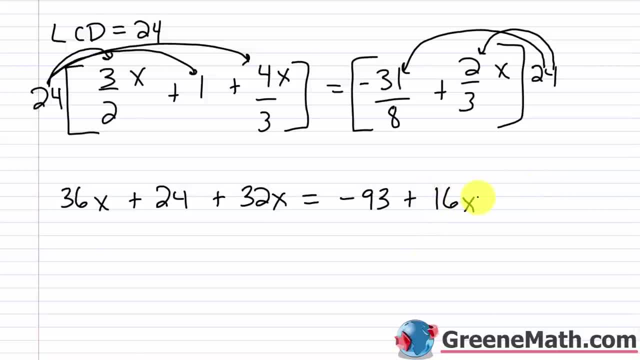 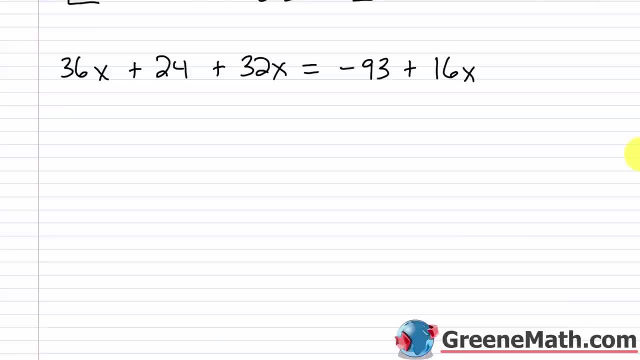 is 16x. okay, so now we're free of fractions. now i just go about my usual business, which is to simplify the left and the right side. so this over here, 36x and 32x, we can combine like terms. that's going to give us 68x. so 68x plus 24 equals over here. i really can't do anything, i just have. 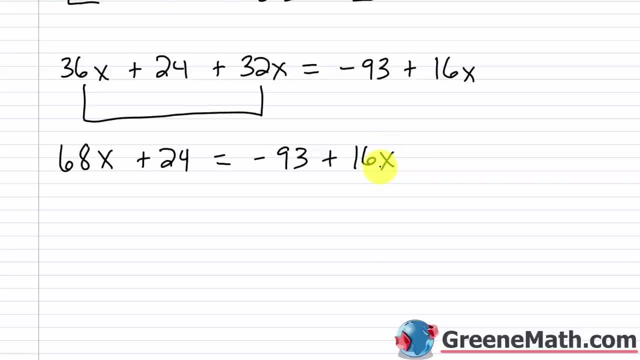 negative 93 plus 16x. now, as we learned in previous lessons, we've got to get the variable terms on one side of the equation. i have 16x over here and i have 68x over here, so i need to move one of them. i always move. 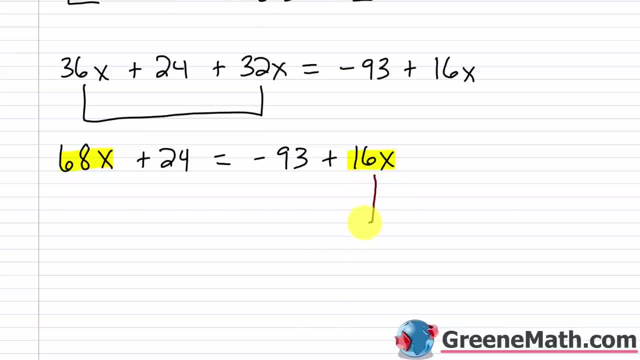 the one on the right to the left. i like my variable to end up on the left, so i'm going to move this over here. and the way i'm going to do that: i'm just going to subtract 16x from both sides of the equation. that'll go away, and then minus 16x over here, 68, minus 16x over here, and 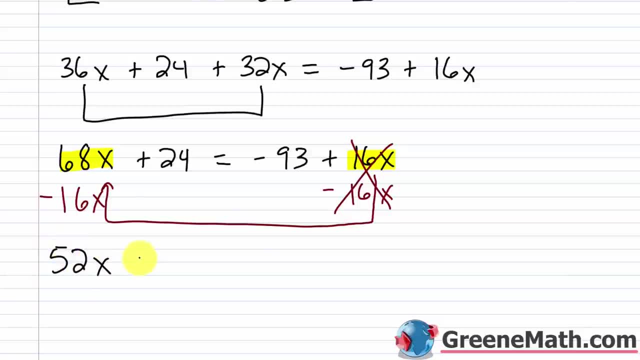 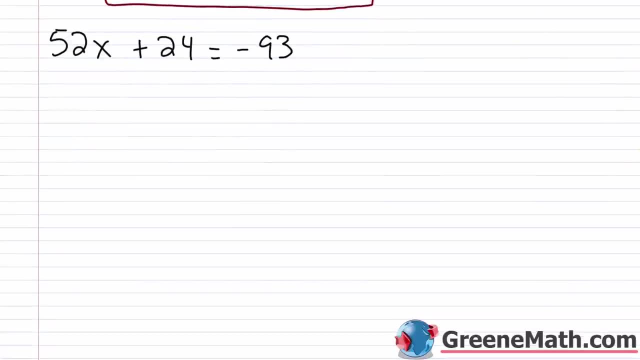 then minus 16x over here, and then minus 16x is 52, so this would be: 52x plus 24 equals negative 93. all right, so now i want to get the variable term by itself, and to get this by itself i need to. 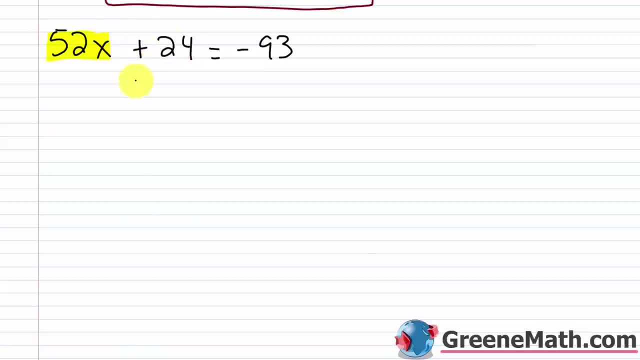 subtract away 24 right, because i have plus 24 over here. that's next to the 52x, so minus 24, minus 24, so that's going to go away. the left side is now just 52x and on the right side, if i have, 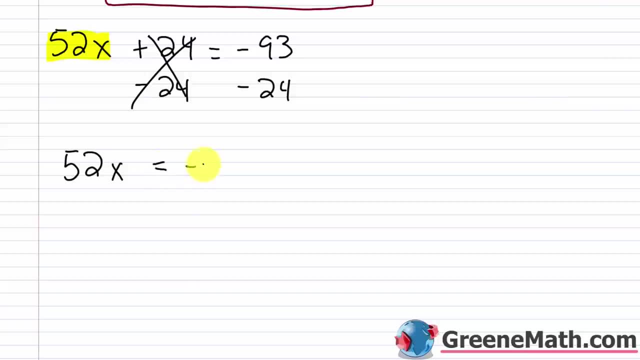 negative 93 minus another 24, i'm going to end up with negative 117. all right, the final step here is to isolate the variable completely and if i look at it, i have what i have: 52 times x. so to get x by itself, i divide by 52, i divide by that coefficient of x. 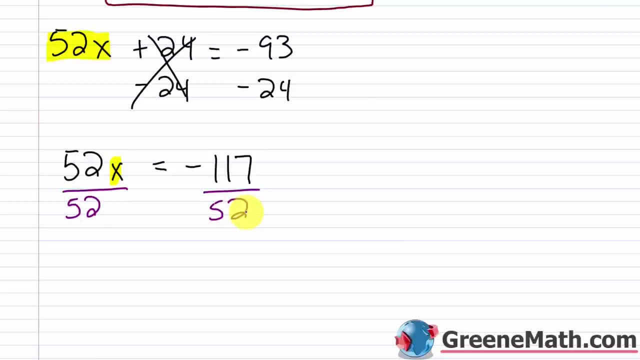 all right, so divide both sides of the equation by 52. this will cancel with this and give me 1. 1 times x is just x, so that's going to be equal to negative 117 divided by 52. so this won't result in an integer or whole number, so we're just going to reduce the fraction. 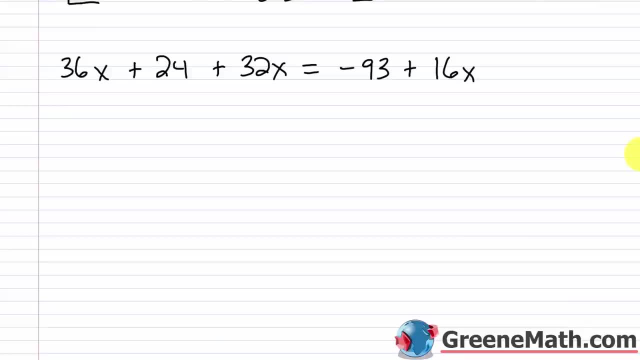 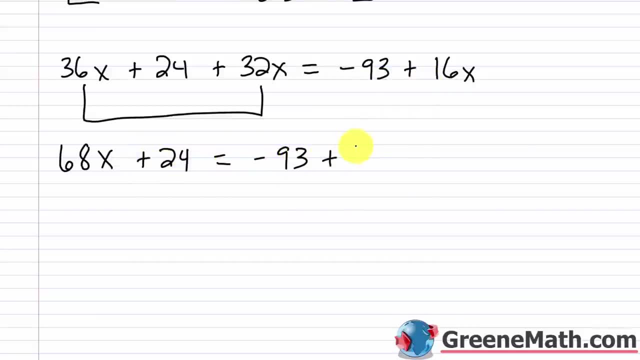 Over here, I really can't do anything. I just have negative 93 plus 16x. Now, as we learned in previous lessons, we've got to get the variable terms on one side of the equation. I have 16x over here. I have 68x over here. So I need to move one of them. I always move the one on the right 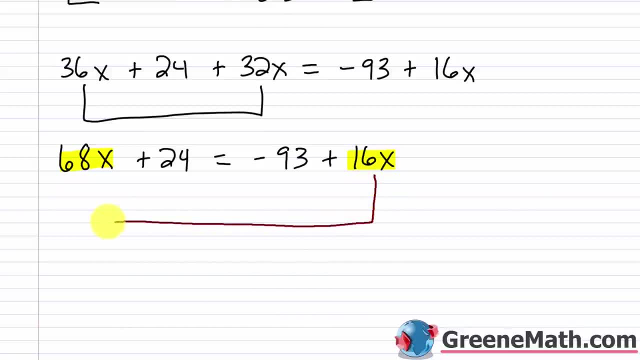 to the left. I like my variable to end up on the left so I'm going to move this over here and the way I'm going to do that I'm just going to subtract 16x from both sides of the equation that'll go away and 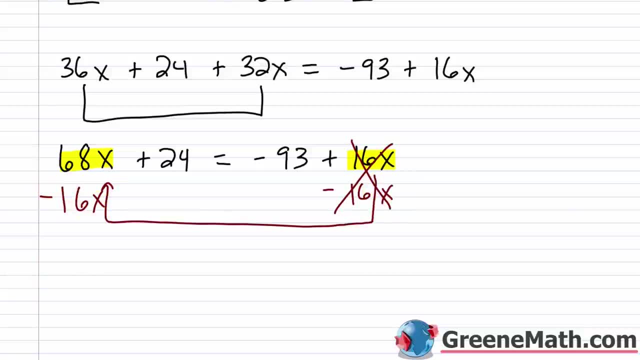 then minus 16x over here 68 minus 16 is 52 so this would be 52x plus 24 equals negative 93 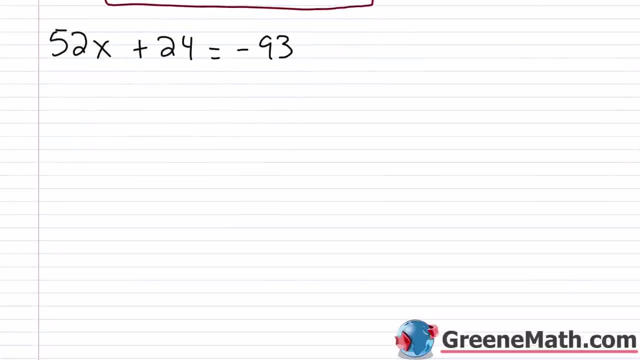 all right so now I want to get the variable term by itself and to get this by itself I need to subtract away 24 right because I have plus 24 over here that's next to the 52x so minus 24 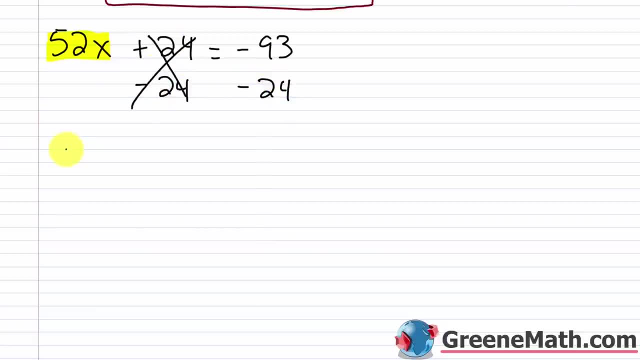 minus 24 so that's going to go away the left side is now just 52x and on the right side if I have negative 93 minus another 24 I'm going to end up with negative 117 all right the final step here 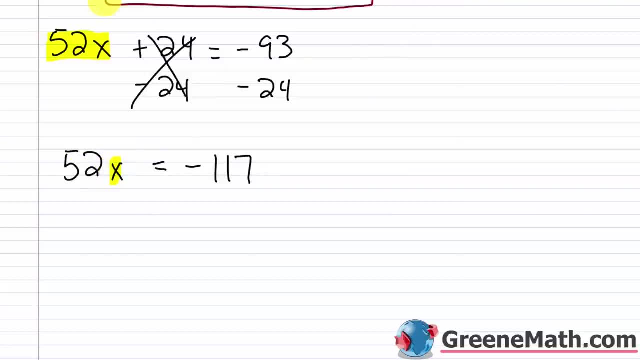 is to isolate the variable completely and if I look at it I have what I have 52 times x so to get x by itself I divide by 52 I divide by 52 times x so I have 52 times x so I have 52 times x by that coefficient of x. All right, so divide both sides of the equation by 52. 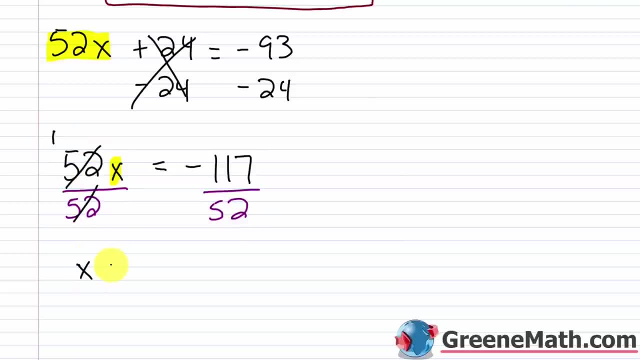 This will cancel with this and give me 1. 1 times x is just x. So that's going to be equal to negative 117 divided by 52. So this won't result in an integer or whole number. 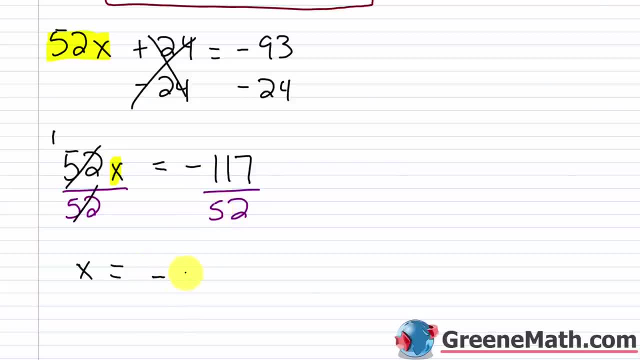 So we're just going to reduce the fraction. So negative 117, I'm going to write negative 1 times 13 times 3 times 3. And for 52, I'm going to write 13 times 2 times 2. So what can I cancel? What can I cancel? I can cancel this 13 with this 13. And I'm really left with what? I'm left with negative 1 times 3 times 3 or negative 9 over 2 times 2 or 4. So my answer here is going to be x equals negative 9 fourths. x equals negative 9 fourths. 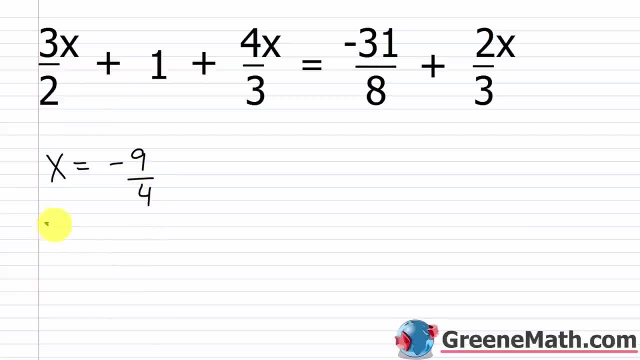 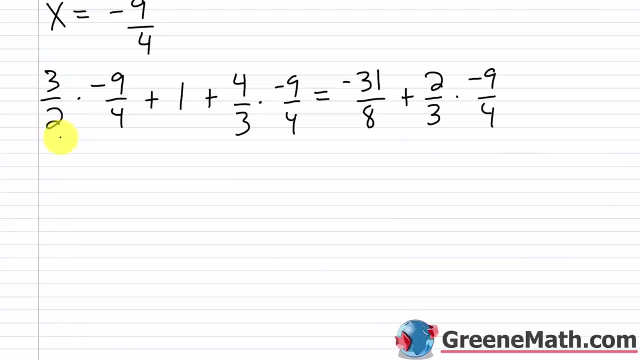 So I'm going to plug in a negative 9 fourths everywhere I see in x. So I'm going to have 3 halves times negative 9 fourths plus 1 plus 4 thirds times negative 9 fourths is equal to negative 31 eighths plus 2 thirds times negative 9 fourths. All right, so if we have 3 halves times negative 9 fourths, what can we cancel? Well, nothing. So we just have to do the multiplication. 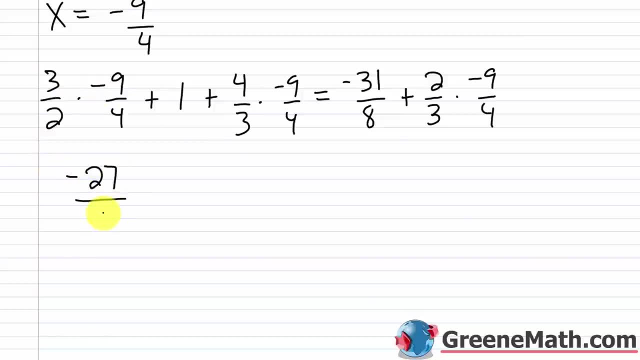 3 times negative 9 fourths. Negative 9 is negative 27. 2 times 4 is 8. So then plus 1 plus over here, this 4 would cancel 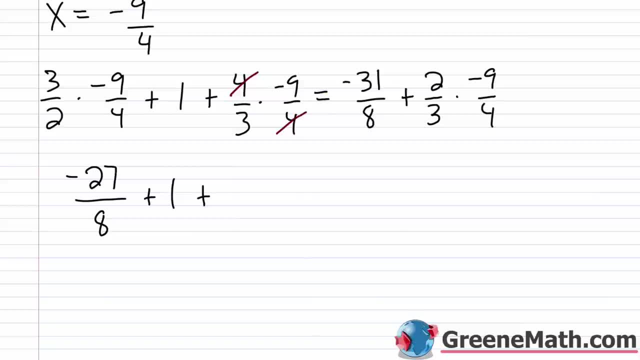 with this 4. And I'd have negative 9 thirds. Negative 9 thirds. And equals, we have negative 31 eighths plus. Over here, I can cancel before I multiply. Negative 9 divided by 3 would be 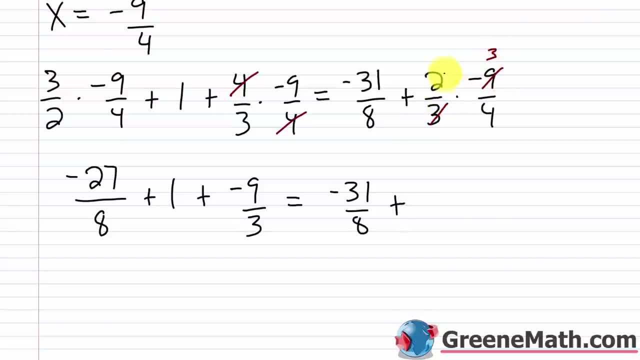 negative 3. So this cancels with this and gives me a 3. And this will cancel with this and give me a 2 down here. 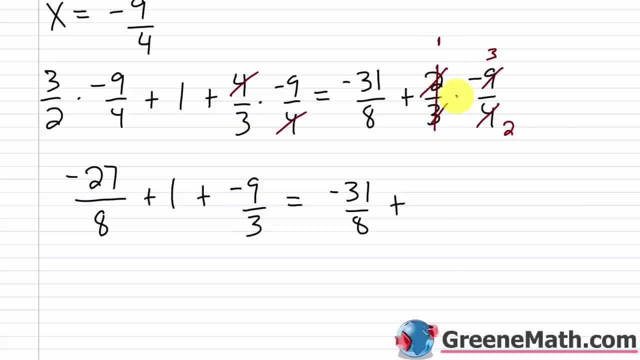 So this completely canceled out. That's just a 1 now. So we'd have basically just negative 3 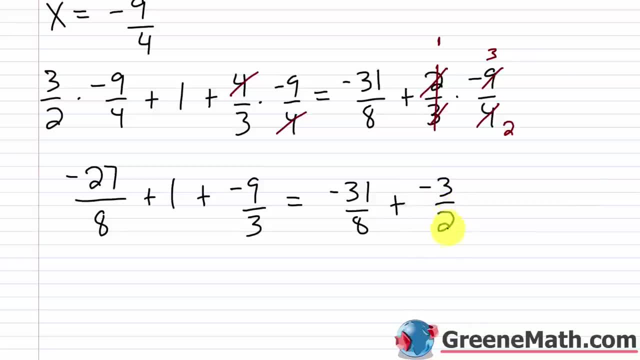 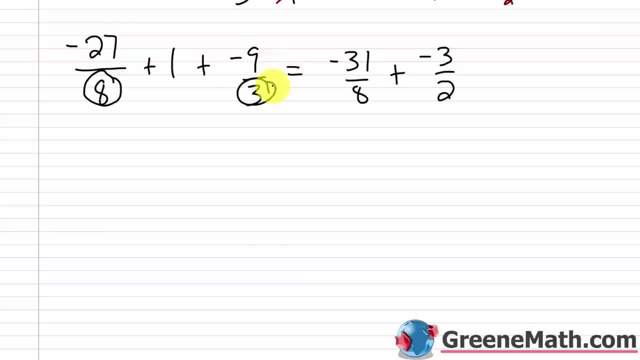 halves. So plus negative 3 halves. All right, so on the left, I got to think about getting a common denominator. So 8 is going to factor into 3 factors of 2. 3 is not going to factor. So the best I can do there for my LCD is going to be 24, right? 8 times 3. So negative 27 over 8 times 3 over 3. Plus, for 1, I'm just going to write it as 24 over 24. It's the same thing as 1. 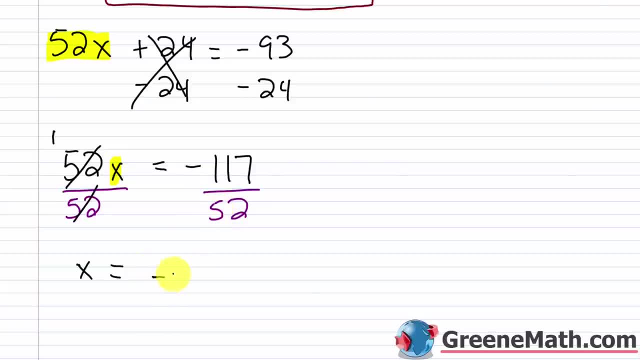 so negative 117, i'm going to write negative 1 times 13 times 3 times 3. and for 52, i'm going to write 13 times 2 times 2. so what can i cancel? what can i cancel? i can cancel this 13 with this. 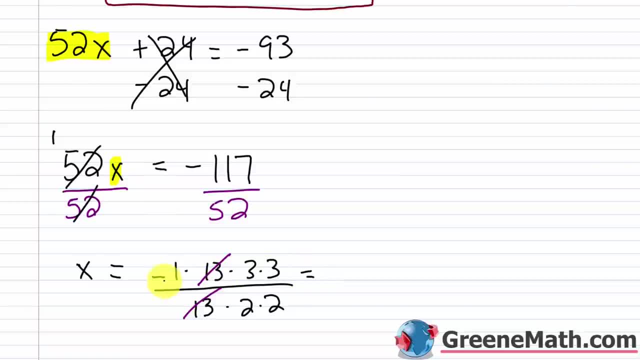 13 and i'm really left with what. i'm left with negative 1 times 3 times 3 or negative 9 over 2 times 2 or 4. so my answer here is going to be that x equals negative 9. fourths, 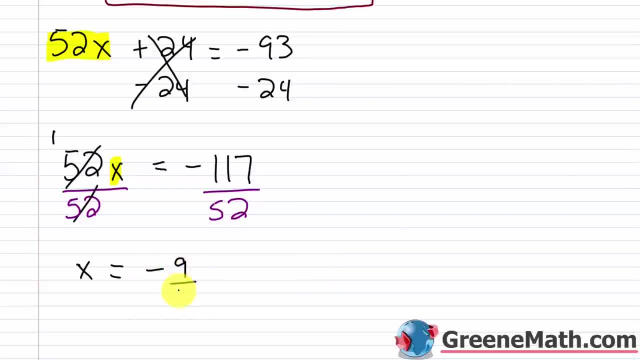 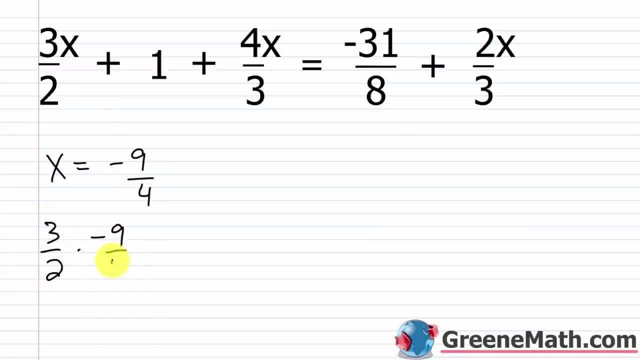 x equals negative 9 fourths, so i'm going to plug in a negative 9 fourths. everywhere i see an x, so i'm going to have three halves times negative 9 fourths plus 1 plus four thirds times negative 9 fourths is equal to negative 31 eighths plus two thirds times negative. 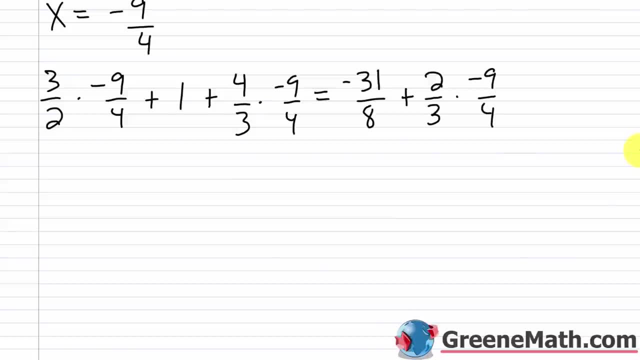 nine fourths, all right. so if we have three halves times negative nine fourths, what can we cancel? well, nothing. so we just have to do the multiplication: three times negative: 9 is negative, 27, 2 times 4 is 8. so then plus 1, plus over here, this 4 would cancel with this 4 and 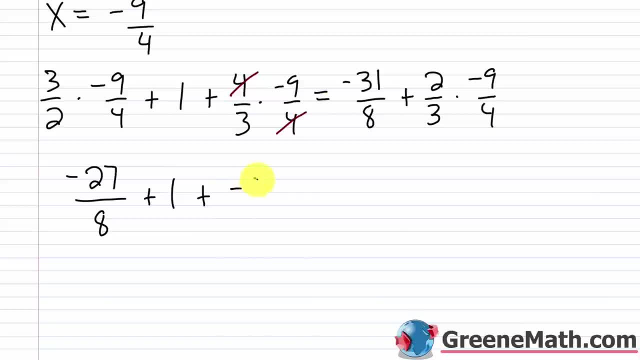 i'd have negative nine thirds. negative nine thirds and equals. we have negative 31 eighths plus over here. i can cancel before i multiply negative 9 divided by 3 would be negative 3, so this cancels with this and gives me a 3, and this will cancel with this and give me a 2 down here. 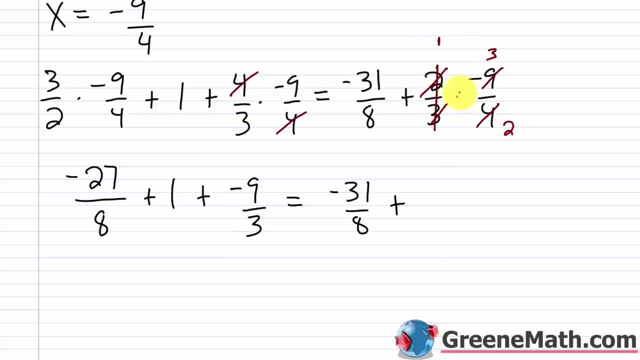 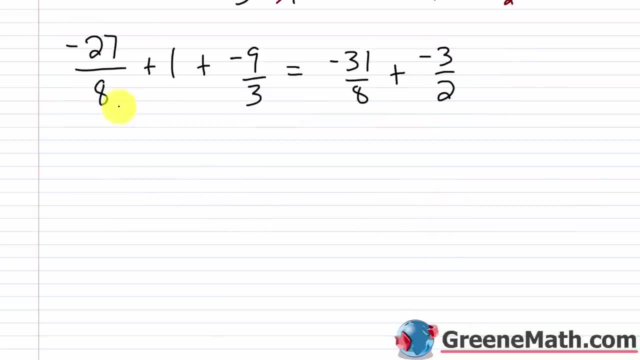 so this completely canceled out. that's just a 1 now, so we'd have basically just negative three halves. so plus negative three halves, all right. so on the left, i gotta think about getting a common denominator. so 8 is going to factor into three factors of 2. 3 is not going to factor, so the best. 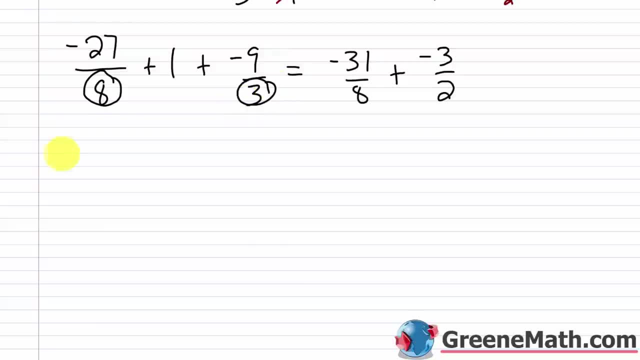 i can do there for my lcd is going to be to get a common denominator. so i'm going to get a common to be 24, right, 8 times 3.. So negative, 27 over 8 times 3 over 3.. Plus for 1,. I'm just going to. 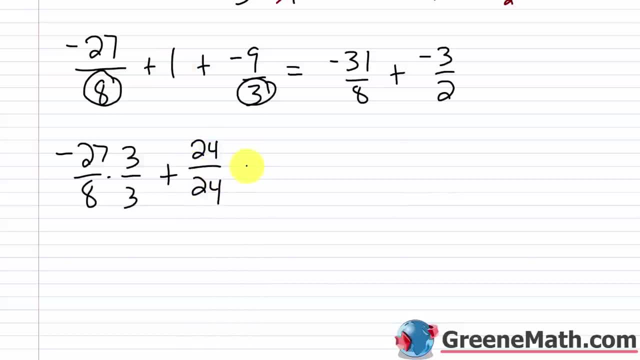 write it as 24 over 24.. It's the same thing as 1.. And then, plus, we'll have negative 9 over 3 times 8 over 8.. Put this equal to negative 31 eighths plus negative 3 halves. All right, So what is? 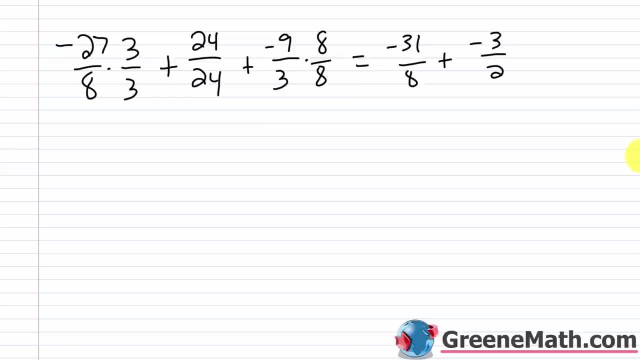 negative 27 times 3?? Well, that's negative 81. So this would be negative 81 over 24 plus 24 over 24, plus negative 9 times 8 is negative 72 over 24.. Let's go ahead and figure this out real quick. 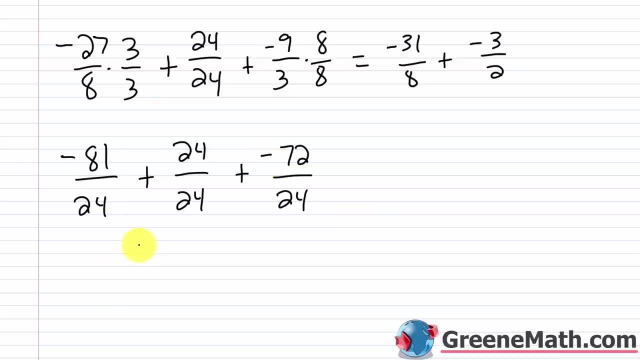 So if I have negative 81 plus negative 72. So 81 plus 72, kind of mentally 1 plus 2- is 3. 8 plus 7 is 15. So that'd be 153 attached to the negative. So that's. 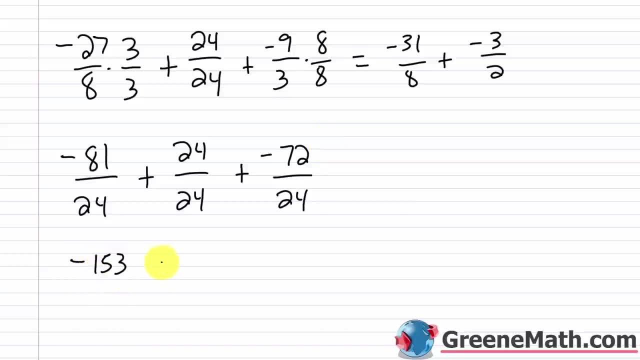 negative: 153 plus 24.. And we can kind of do that in our head also because really think about 153 minus 24.. That's going to give you 129. And then just slap the negative on there. So we would have. 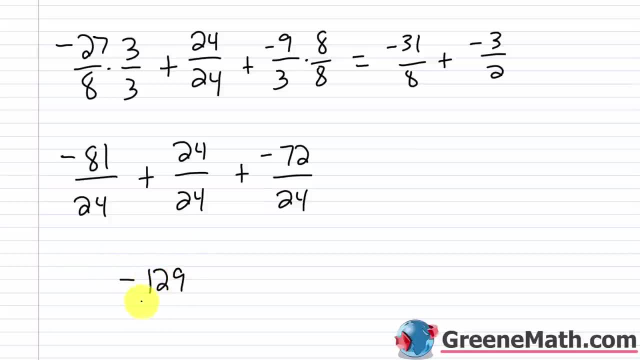 negative, negative, 129 over 24.. So this is equal to: and then over here, really, I can easily see that the LCD is going to be 8. So I just need to multiply this side by 4 over 8.. So I'm going to do that, So I'm going to do that, So I'm going to do that, So I'm going to. 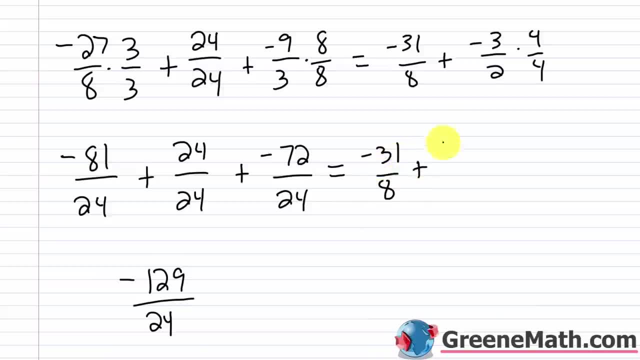 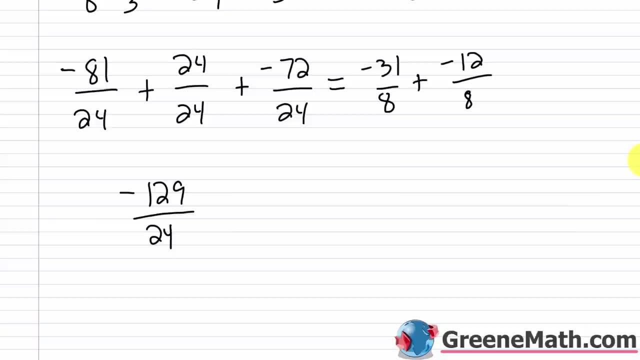 and I'd have negative 31 eighths plus negative 3 times 4 is negative 12. over 2 times 4 is 8.. So negative 31 plus negative 12 is going to be negative 43. So we'll have equals negative 43 eighths. 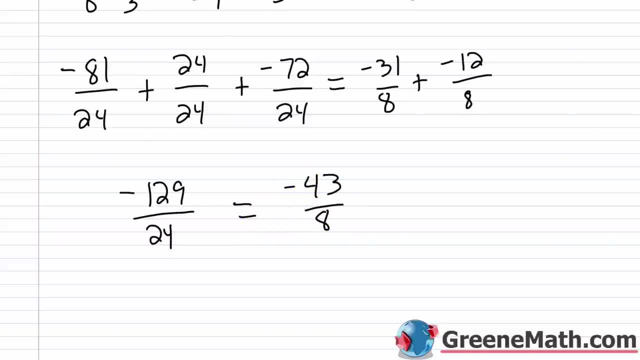 So a lot of you at this point will stop and go: okay, I got the wrong answer. What happened? Always, make sure that when you get fractions, they're reduced to their lowest terms or they're simplified. These fractions are the same. The one on the left is just not simplified. If I think about negative 129, I can write this: 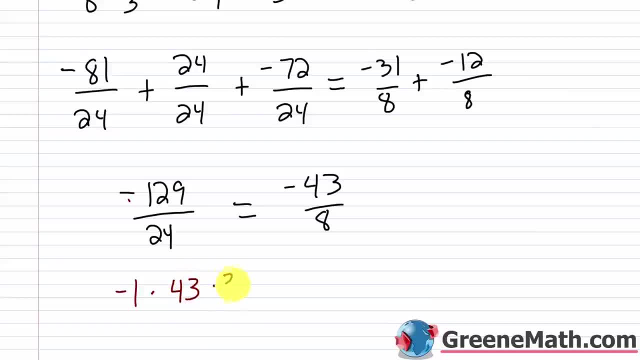 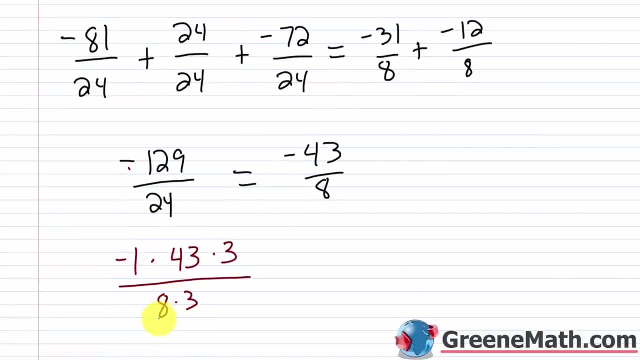 as negative 1 times 43 times 3.. I can write 24 as 8 times 3. And we can see that we can cancel this 3 with this 3. And I'm left with negative 1 times 43 or negative 43 over 8. That's what I. 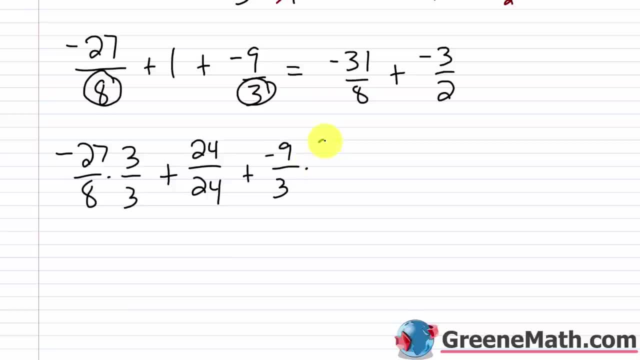 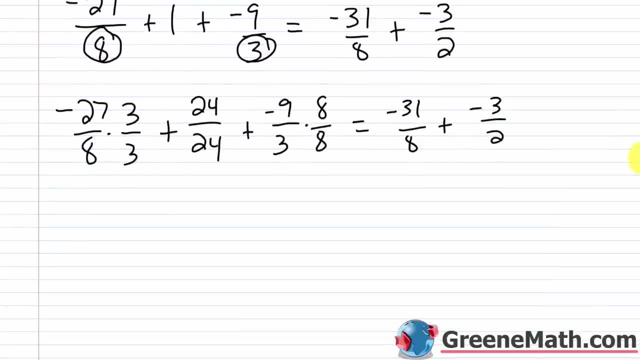 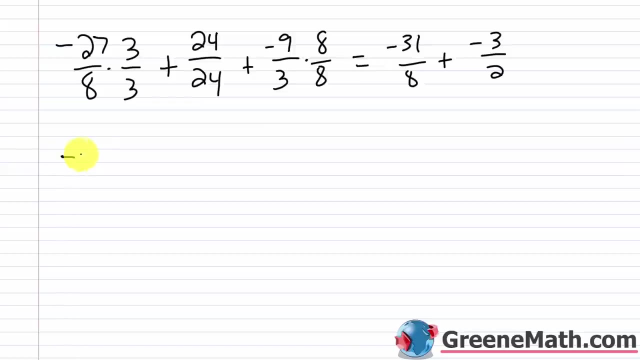 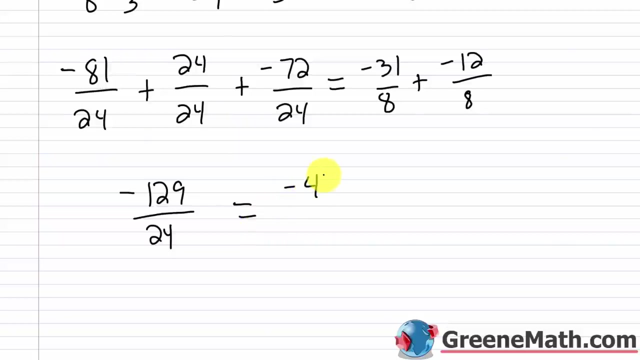 And then plus, we'll have negative 9 over 3 times 8 over 8. Put this equal to negative 31 eighths plus negative 3 halves. All right. So what is negative 27 times 3? Well, that's negative 81. So this would be negative 81 over 24 plus 24 over 24 plus negative 9 times 8 is negative 72 over 24. Let's go ahead and figure. This out real quick. So if I have negative 81 plus negative 72. So 81 plus 72, kind of mentally, 1 plus 2 is 3. 8 plus 7 is 15. So that'd be 153 attached to the negative. So that's negative 153 plus 24. And we can kind of do that in our head also, because really think about 153 minus 24. That's going to give you 129. And then just slap the negative on there. So we would have negative negative 129 over 24. So this is equal to. And then over here, really, I can easily see that the LCD is going to be 8. So I just need to multiply this side by 4 over 4. And I'd have negative 31 eighths plus negative 3 times 4 is negative 12 over 2 times 4 is 8. So negative 31 plus negative 12 is going to be negative 43. So we'll have equals negative 43 eighths. 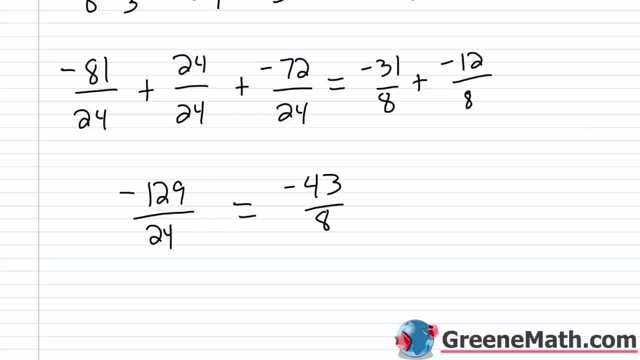 So a lot of you at this point will stop and go, OK, I got the wrong answer. What happened? 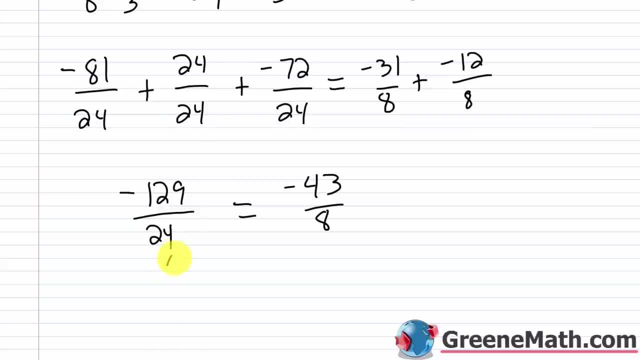 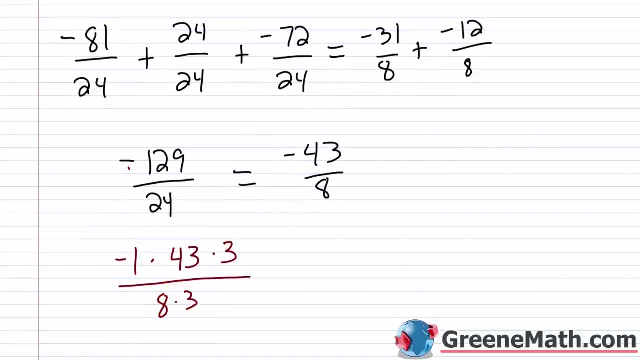 Always make sure that when you get fractions, they're reduced to their lowest terms or they're simplified. These fractions are the same. The one on the left is just not simplified. If I think about negative 129, I can write this as negative 1 times 43 times 3. I can write 24 as 8 times 3. And we can see that we can cancel. This 3 with this 3. And I'm left with negative 1 times 43 or negative 43 over 8. That's what I have over here, negative 43 over 8. And you can't simplify that any further on either side. It doesn't matter because you've got the same number on either side. But if you wanted to think, OK, well, can I simplify this further just for the sake of completeness? You can't because 8 is 2 times 2 times 2. And negative 43 is not divisible by 2. So you'll end up with negative 43 eighths equals negative 43 eighths. 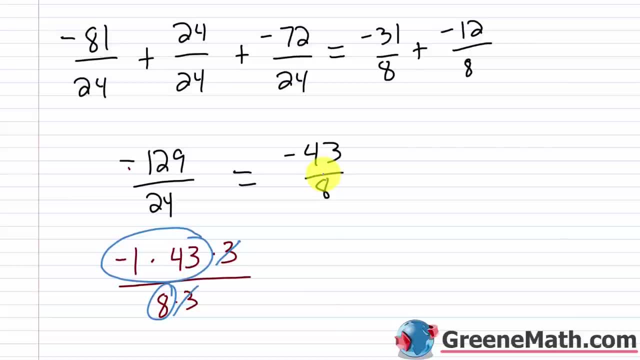 have over here negative 43 over 8. And you can't simplify that any further. right on either side, It doesn't matter because you've got the same number on either side. But if you wanted to think, OK, well, can I simplify this further just for the sake of completeness, You can't right, Because 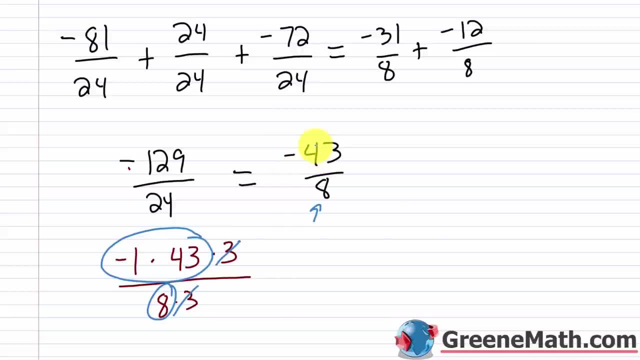 8 is 2 times 2 times 2.. And negative 43 is not divisible by 2.. So you'll end up with negative 43 eighths equals negative 43 eighths, And so you know your solution, which we found was x equals. 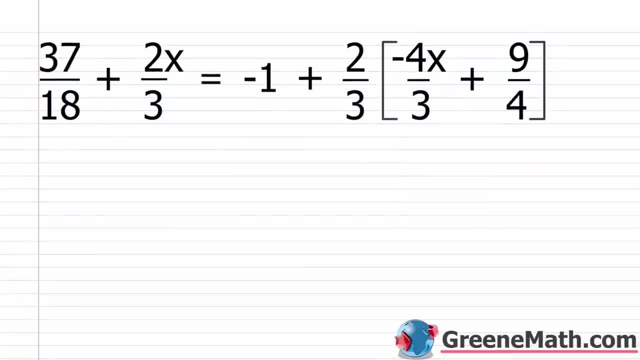 negative 9 fourths is correct. All right, let's take a look at another type of problem you're going to come across. So we have 37 eighteenths plus 2 thirds x Equals negative 1 plus 2 thirds times this quantity: negative 4 thirds x plus 9 fourths. 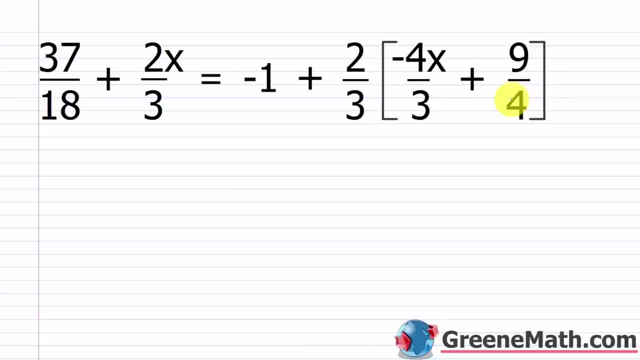 If I begin my problem the normal way, if I say, OK, what's the LCD of all the fractions involved, And I go to multiply it, it's not going to clear all the fractions right away. What you need to do is use your distributive property first. So if you come across a problem where you have fractions, 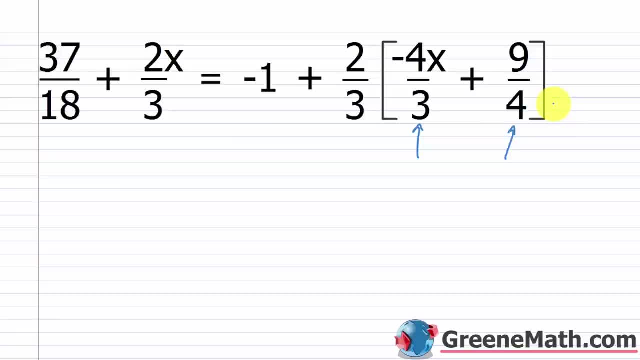 that are inside of a set of parentheses or a set of brackets. use the distributive property first and simplify. So what I want to do. so I have 37 eighteenths over here plus two thirds. x equals negative 1 plus I'm going to remove the brackets two thirds times. 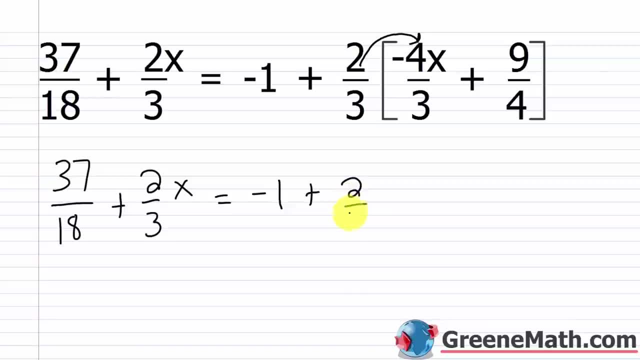 negative four thirds x. I'm going to have two thirds times negative, four thirds x. So 2 times negative, 4 is negative 8.. 3 times 3 is 9.. So this would be negative 8 ninths. So I'm going to put: 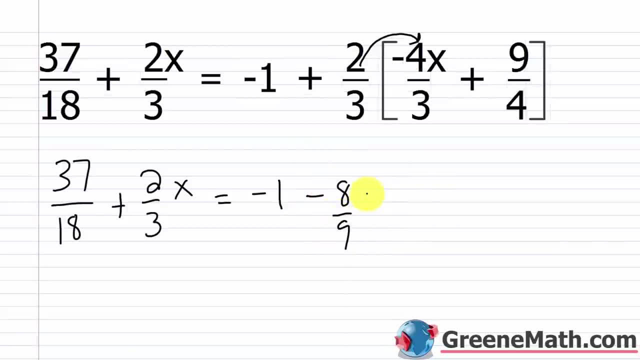 minus minus eight ninths times x, and then again two thirds times nine fourths. so two thirds times nine fourths, and what i can go ahead and do is cancel this with this. that'll give me a three. cancel this with this, and that'll give me a two. so this is canceled completely. it's just a one. 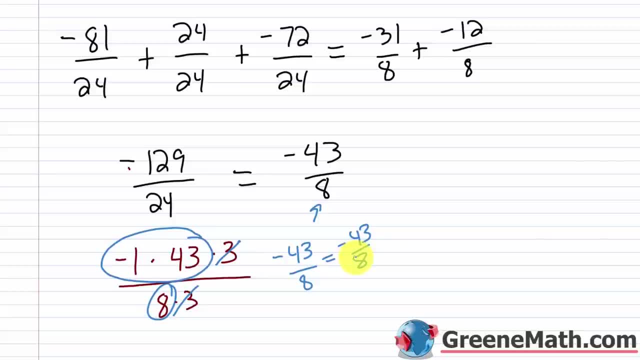 So you know your solution, which we found was x equals negative 9 fourths is correct. All right, 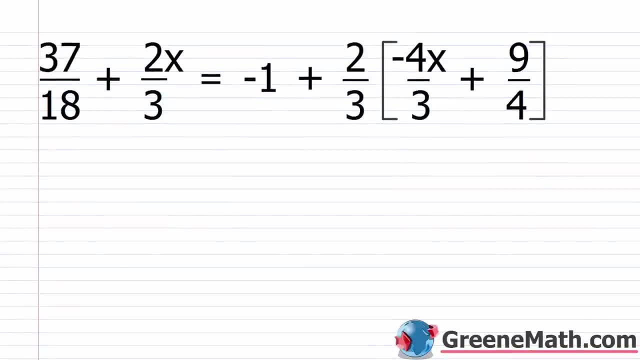 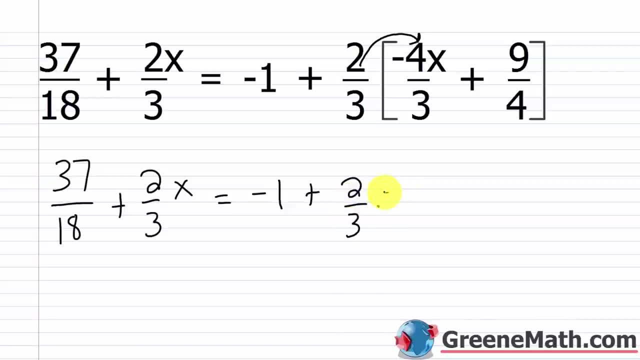 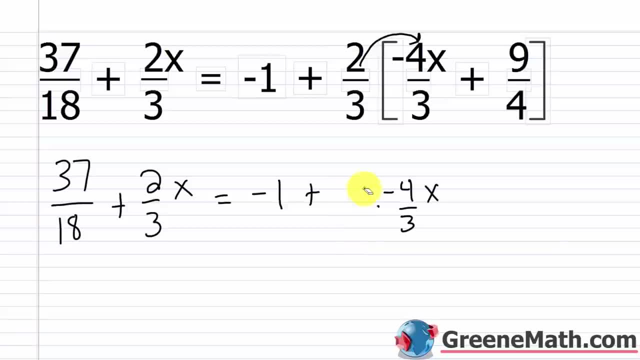 3 times 3 is 9. So this would be negative 8 ninths. So I'm going to put minus 8 ninths 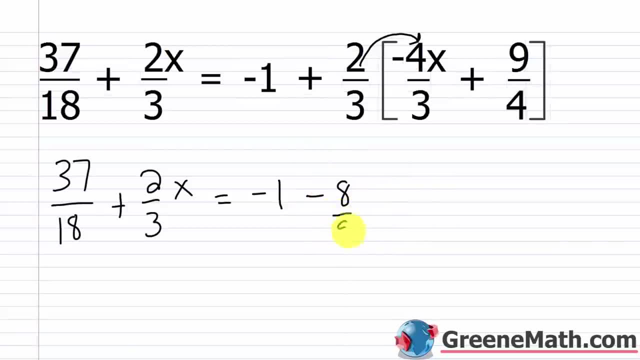 times x and then again, 2 thirds times 9 fourths. So 2 thirds times 9 fourths 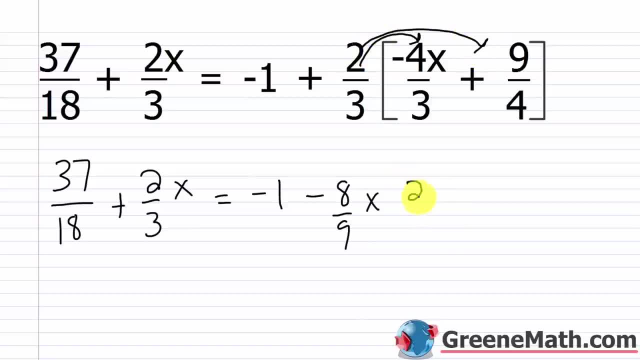 and what I can go ahead and do is cancel this cancel this with this. That will give me a 3. Cancel this with this approximately. 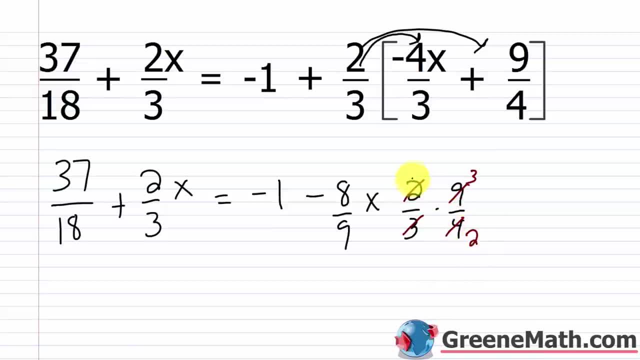 If I come across an query that says, can 2 thirds of x times 9 and 8 táthos could be the answer, without even naming it, this. And that'll give me a two. So this is canceled completely. It's just a one. And so I'll 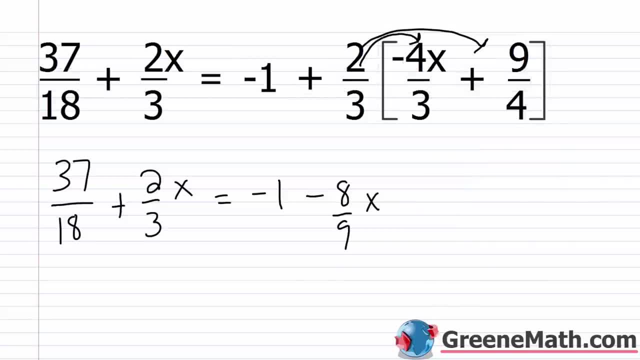 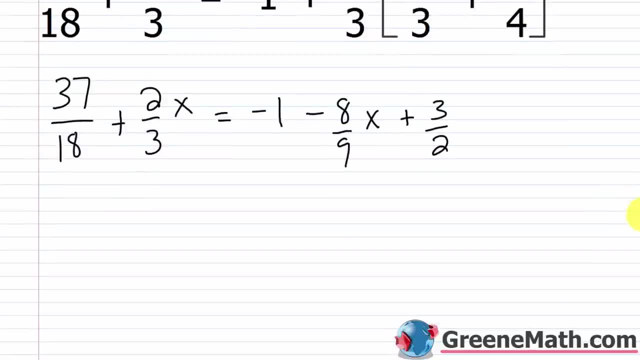 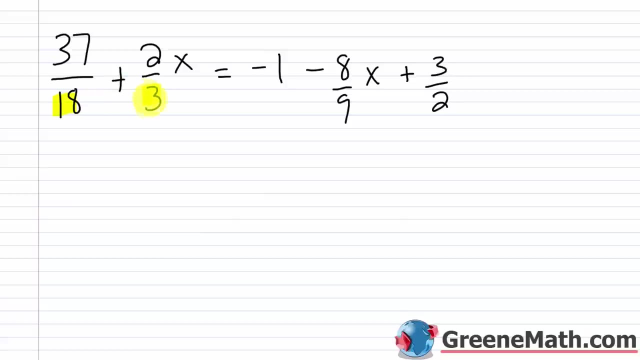 have three halves there. So this will be plus, plus three halves. Okay. So once you've done that, go ahead and think about, okay, what's the LCD now? So I have 18. I have three, I have nine, and I have two. And at this point in your math career, you should be able to kind of look at that and say, okay, I know the LCD is 18, right? So I know most of you can do that. If you can't, 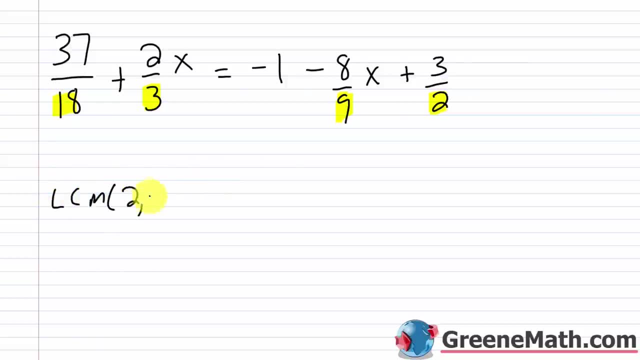 again, take the steps. So LCM of two, three, nine, and 18. So I know that two doesn't factor. 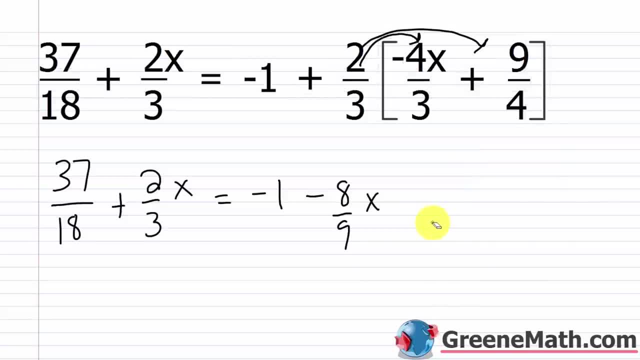 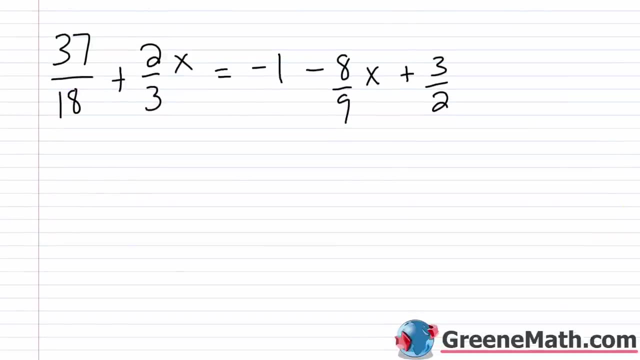 and so i'll have three halves there. so this will be plus plus three halves, okay. so once you've done that, go ahead and think about: okay, what's the lcd now? so i have 18, i have three, i have nine and i have two, and at this point in your math career you should be able to kind of look at that and say okay. 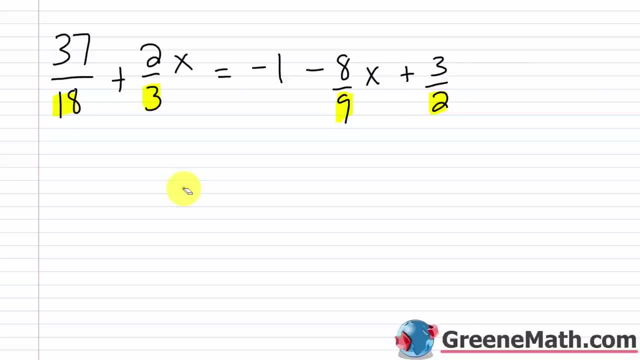 i know the lcd is 18, right, so i know most of you can do that if you can't again take the step. so lcm of two, three, nine and 18. so i know that two doesn't factor, i know that three doesn't factor. nine is three times three, so i'm only going to put one more copy of three in there, because nine 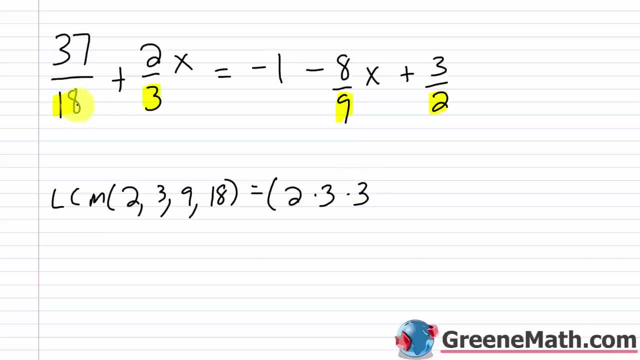 is three times three. i don't want the largest number of repeats to go in. 18 is two, which i already have in there. times three, which is already in there. times three again. you could think about it as two times nine or, you know, three times six. however you want to do it, it's going to break. 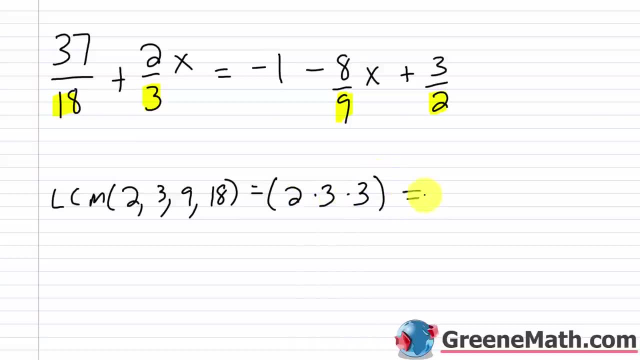 down into two times three times three, and we already have that there. so if we multiply we get 18, so that's the lcm of those numbers, and so for the lcd it's 18. all right, so now we're just going to multiply both sides of the equation by 18. again, you want to use brackets or parentheses? 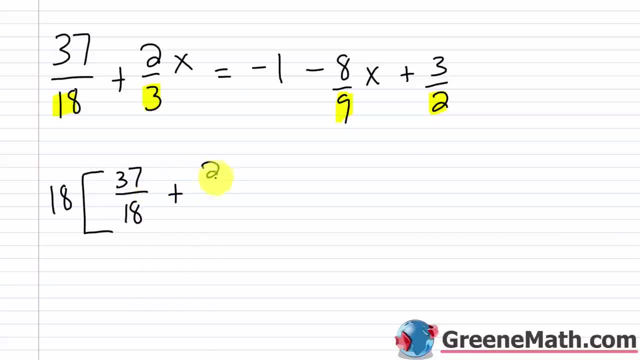 make sure that you multiply each term by 18, all right. so over here on the left, if i do 18 times 37, 18th, we know that 18 would cancel with 18, right? so this would just be 37. then plus, we have 18 times two-thirds x 18 would cancel with. 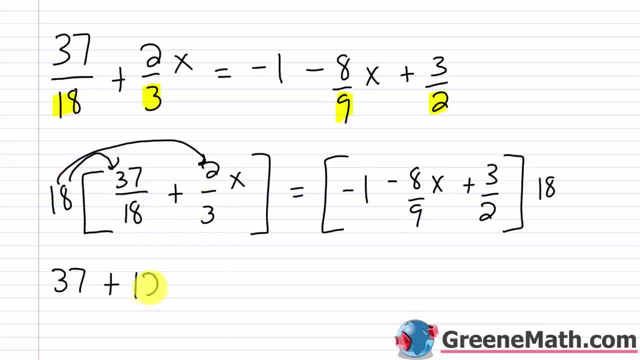 3, giving me a 6. 6 times 2 is 12, so this would be 12: x and this equals: over here: 18 times negative. 1 is negative. 18 over here: 18 times negative. 1 is negative. 18 over here: 18 times negative. 1 is negative. 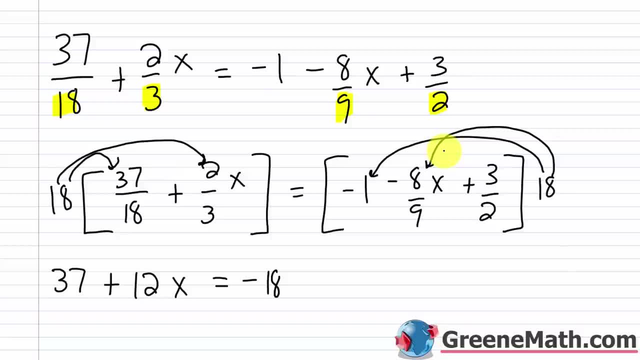 8. ninths, think about 18. canceling with 9 and giving me a 2, 2 times negative 8 is negative 16, so this would be negative 16 times that variable x, then plus lastly, i have 18 times 3 halves. 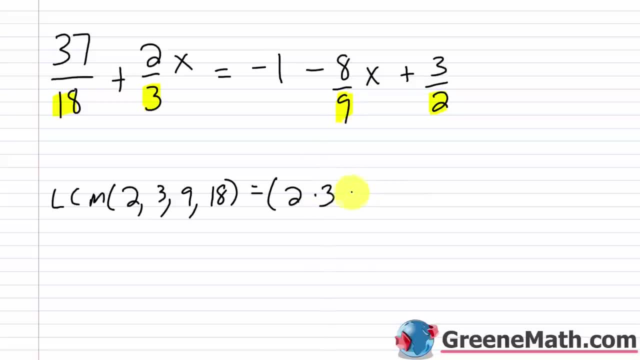 I know that three doesn't factor. Nine is three times three. So I'm only going to put one more copy of three in there because nine is three times three. I don't want the largest number 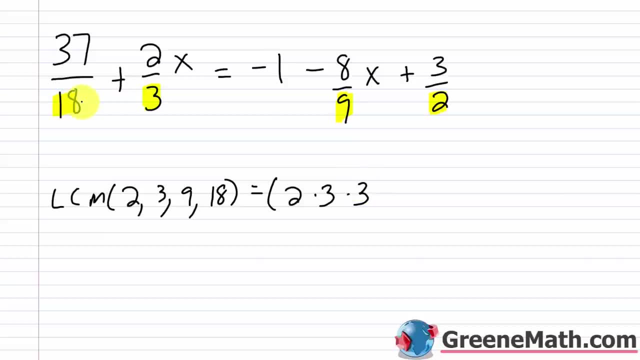 of repeats to go in. 18 is two, which I already have in there, times three, which is already in there. So I'm only going to put one more copy of three in there because nine is three times three. 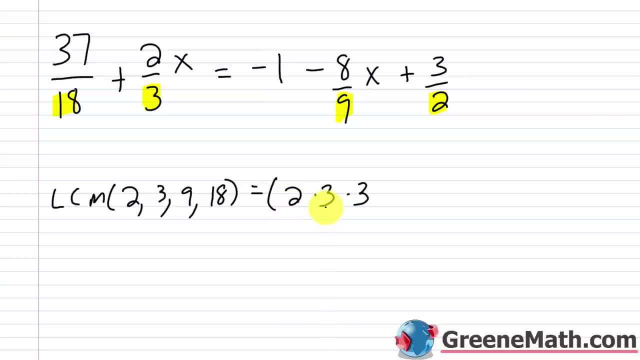 Times three again. You could think about it as two times nine or three times six. However you want to do it, it's going to break down into two times three times three. And we already have that there. So if we multiply, we get 18. So that's the LCM of those numbers. And so for the LCD, 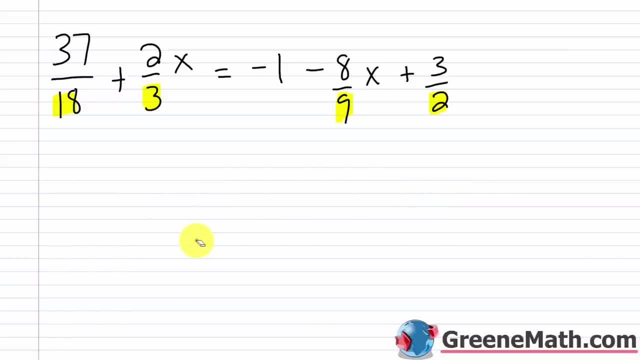 it's 18. All right. So now we're just going to multiply both sides of the equation by 18. Again, you want to use brackets or parentheses. Make sure that you're not going to have to do that. So you're going to have to do that. You multiply each term by 18. 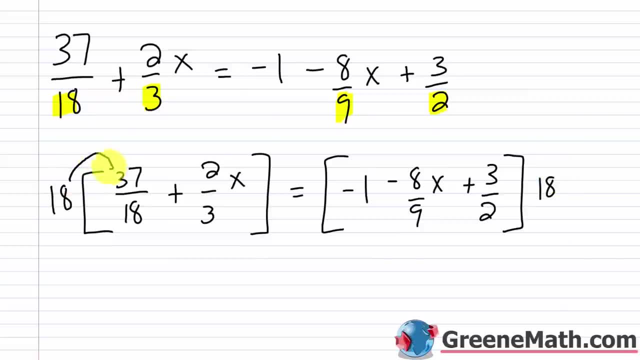 All right. So over here on the left, if I do 18 times 37 18ths, we know that 18 would cancel with 18, right? So this would just be 37. Then plus, we have 18 times two thirds x. 18 would cancel with three, giving me a six. Six times two is 12. So this would be 12x. And then we're going to multiply each term by 18. So this would just be 37. So this would be 12x. And this equals, over here, 18 times negative one is negative 18. Over here, 18 times negative eight ninths. Think about 18 canceling with nine and giving me a two. Two times negative eight is negative 16. So this would be negative 16 times that variable x. 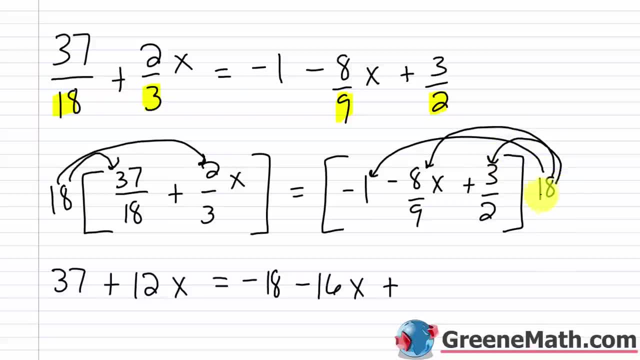 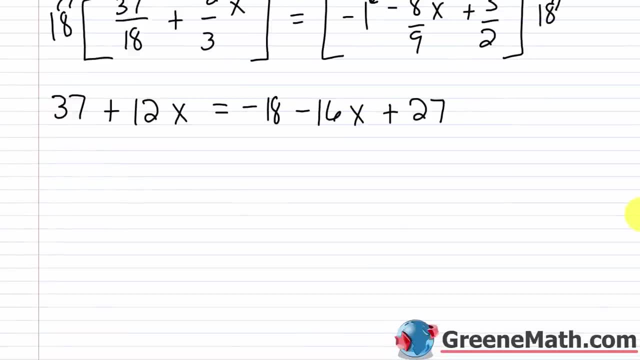 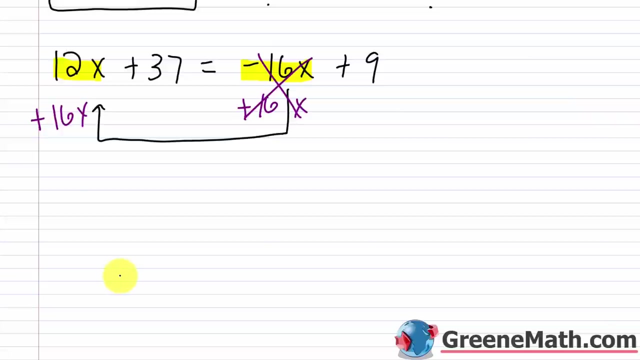 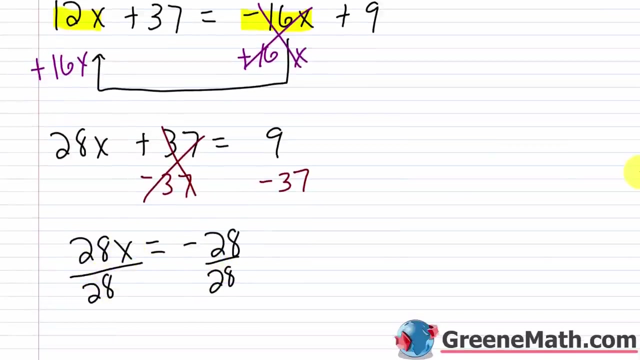 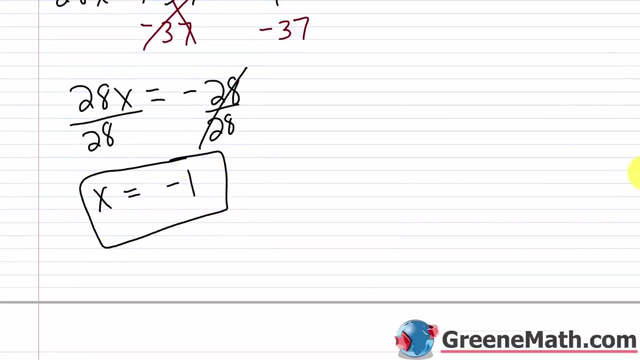 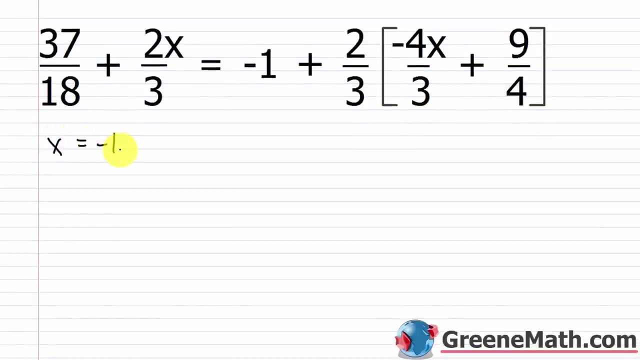 Then plus, lastly, I have 18 times three halves. 18 would cancel with two and give me a nine. Nine times three is 27. Okay. Now we just simplify. So I can't do anything to the left, I'm going to do anything to the left I'm just going to copy that down so 12x plus 37 I'm just going to reverse the order on the right I can simplify because I can add negative 18 and 27 that's going to give me positive 9 so I'd have negative 16x plus 9 I want all my variable terms on one side of the equation so because I have one there and one here I always like my variable on the left I'm going to move that guy over there so I'm going to add 16x to both sides of the equation so that's going to go away 12x plus 16x is 28x so plus 37 equals 9 I'm going to get my variable term by itself on the left so that means I'm going to be subtracting away the 37 from both sides of the equation so that's gone so I'll have 28x equals what is 9 minus 37 that's going to be negative 28 and we divide both sides of the equation by 28 the coefficient of x in order to isolate the variable completely and I'm going to have x is equal to negative 1 okay x is equal to negative 1 all right so we could erase all this and check so x again equals negative 1 so we'd have 37 18ths plus 2 times negative 1 which is just negative 2 so I'm just going to write minus two-thirds and this is equal to 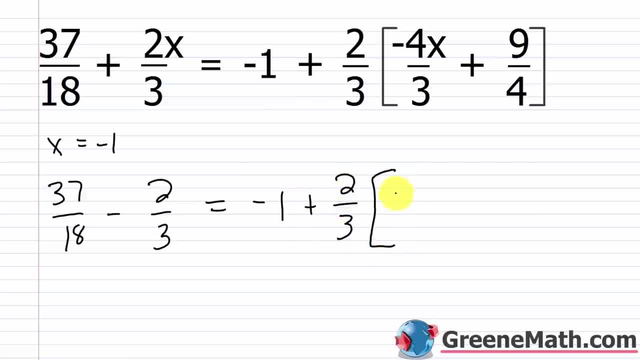 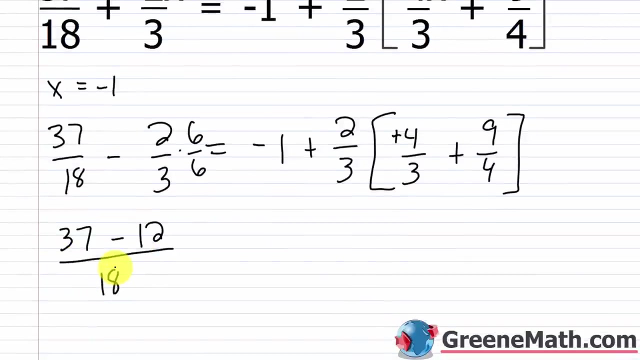 negative 1 plus two-thirds times this quantity will have negative 4 times negative 1 so that's positive 4 over 3 plus 9 fourths so on the left side I just multiply this by 6 over 6 and I'll have a common denominator right so I'd have 37 minus 2 times 6 is 12 over the common denominator of 18 37 minus 12 is 25 so this would be 25 over 18 25 over 18 so I'd have 37 minus 2 times 6 is 25 over the common denominator of 18 so this would be 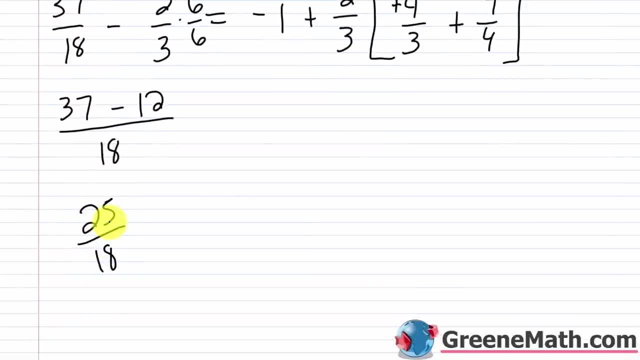 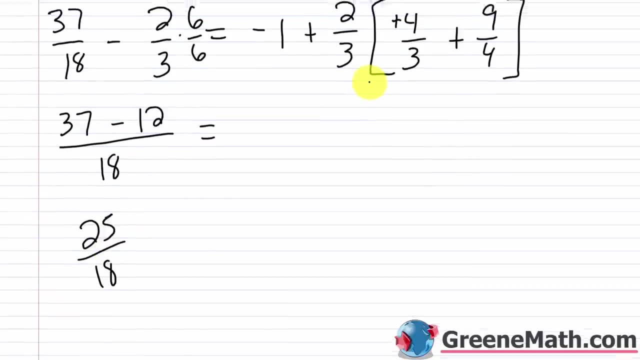 25 over 18, and 25 is 5 times 5, 18 we know is 2 times 3 times 3, so really we can't make that any more simple. Over here, if I think about 4 thirds plus 9 fourths, I'd multiply this by 4 over 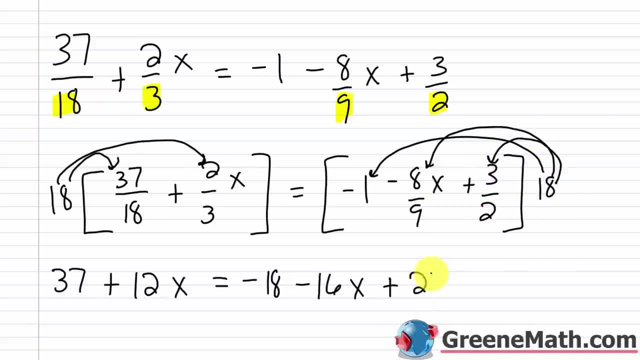 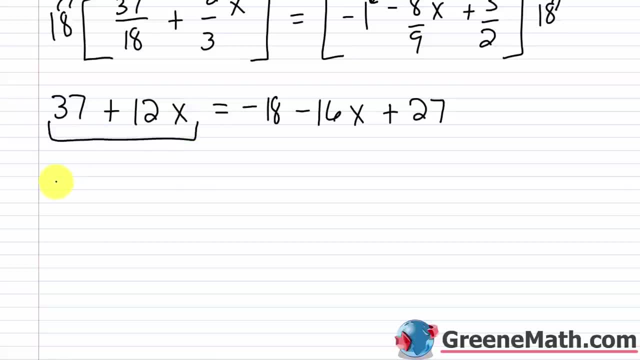 18 would cancel with 2 and give me a 9. 9 times 3 is 27. okay, now we just simplify. so i can't do anything to the left, i'm just going to copy that down. so 12 x plus 37. i'm just going to reverse. 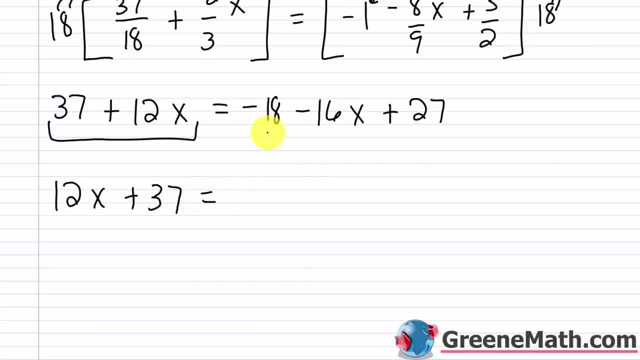 the order on the right hand side. i'm just going to copy that down. so 12 x plus 37. i'm just going to reverse the order on the right. i can simplify because i can add negative 18 and 27. that's going to give me positive 9. so i'd have negative 16 x plus 9. i want all my variable terms on one side. 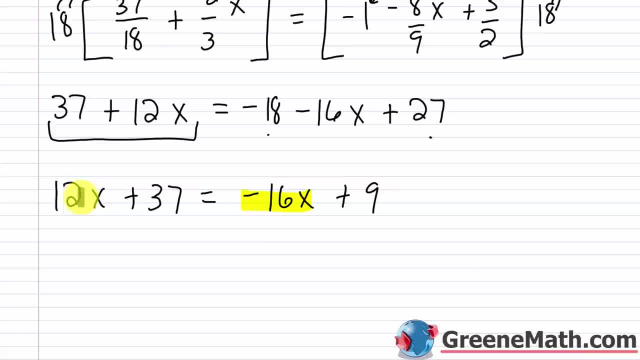 of the equation. so because i have one there and one here, i always like my variable on the left- i'm going to move that guy over there. so i'm going to add 16 x to both sides of the equation. so that's going to go away. 12 x plus 16 x is 28 x. 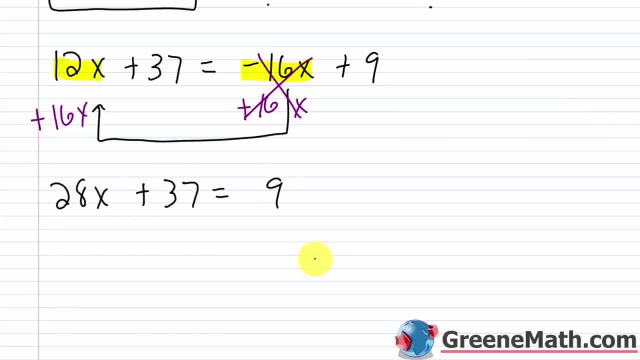 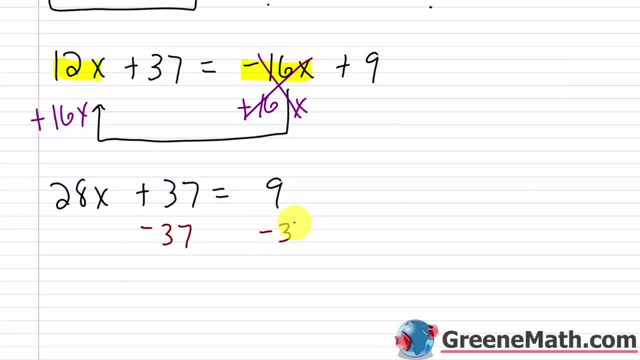 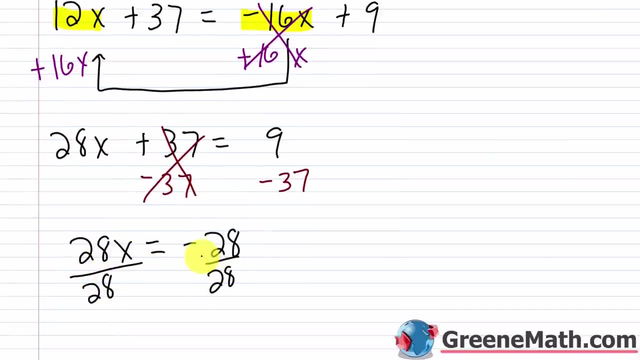 subtracting away the 37 from both sides of the equation. so that's gone. so i'll have 28. x equals what is 9 minus 37. that's going to be negative 28. and we divide both sides of the equation by 28, the coefficient of x, in order to isolate the variable completely, and i'm going to have x- is 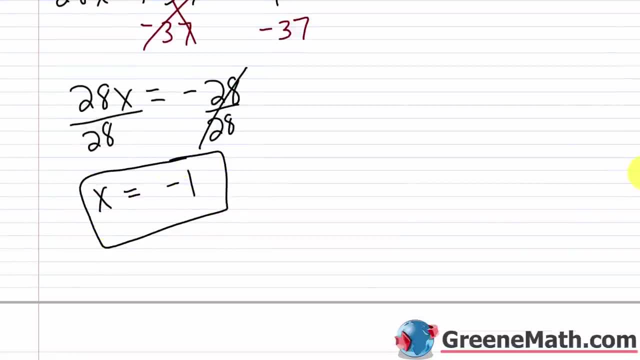 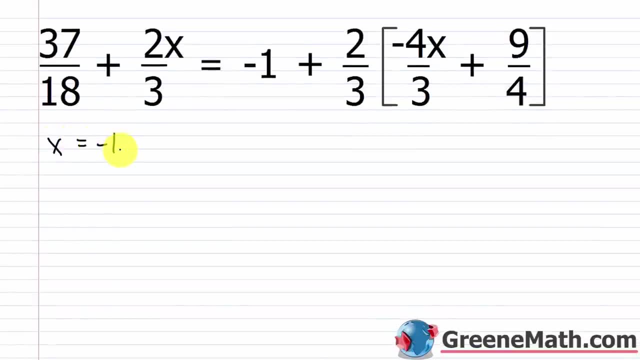 equal to negative 1. okay, x is equal to negative 1. all right, so we could erase all this and check. so x again equals negative 1. so we'd have 37 18ths plus 2 times negative 1, which is just negative 2. so i'm just 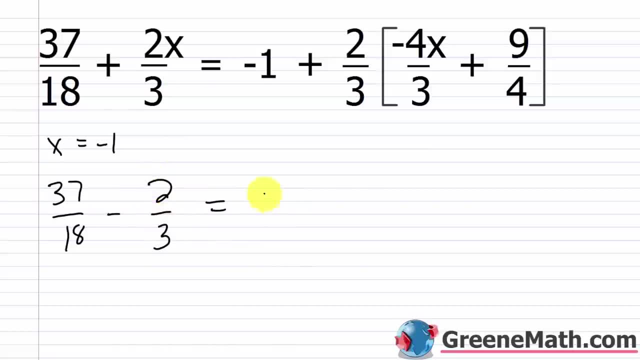 going to write minus two-thirds, and this is equal to negative 1 plus two-thirds times. this quantity will have negative 4 times negative 1, so that's positive 4 over 3 plus 9 fourths. so on the left side, i just multiply this by 6 over 6 and i'll have a common denominator. 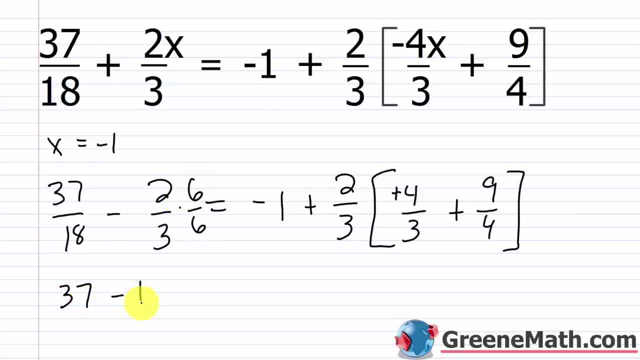 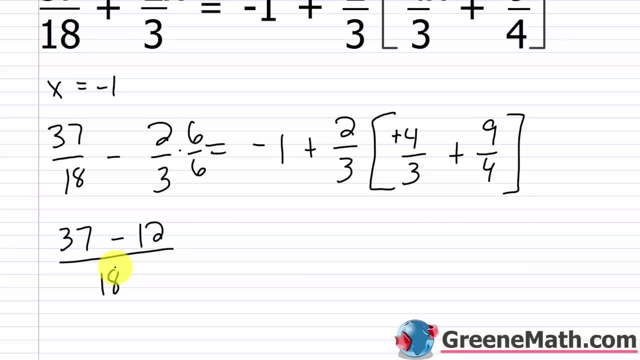 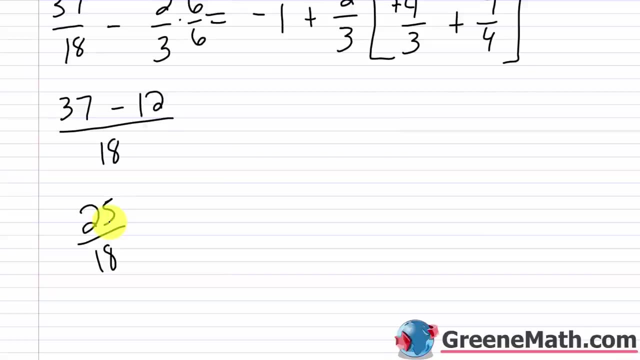 right. so i'd have: 37 minus 2 times 6 is 12 over the common denominator of 18. 37 minus 12 is 25, so this would be 25 over 18, 25 over 18 and 25 is 5 times 5. 18, we know, is 2 times 3 times 3, so really, 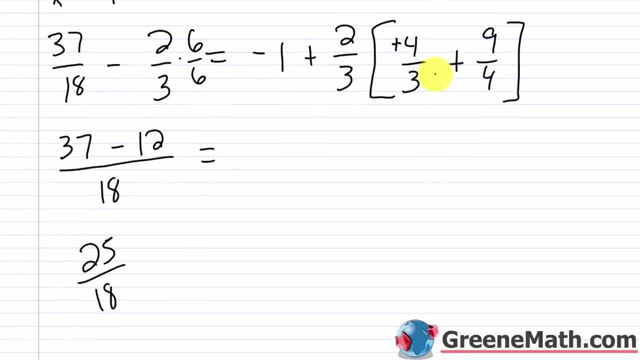 we can't make that any more simple over here. if i think about 4 thirds plus 9 fourths, i'd multiply this by 4 over 4. i multiply this by 3 over 3 and so negative 1 plus 2 thirds times 4 times 4 is 16 over 12. plus 9 times 3 is 27 over 12 and 16 plus 27 would be 43, so i'd have 43 twelfths. so let me just erase this and write 43 twelfths. 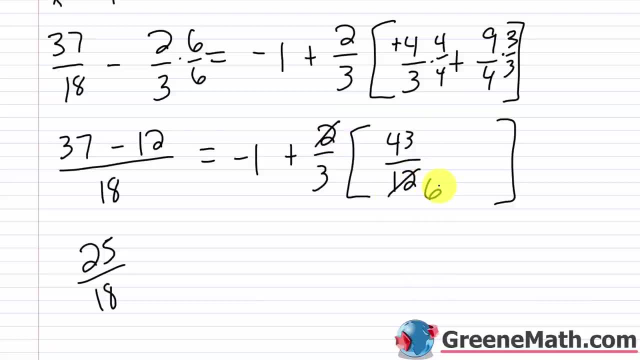 so if i'm multiplying here, this is going to cancel with this and give me a 6, and so what i'm going to have is negative 1 plus i'll have 1 times 43, or 43 over, 3 times 6 or 18.. so to get a common denominator, 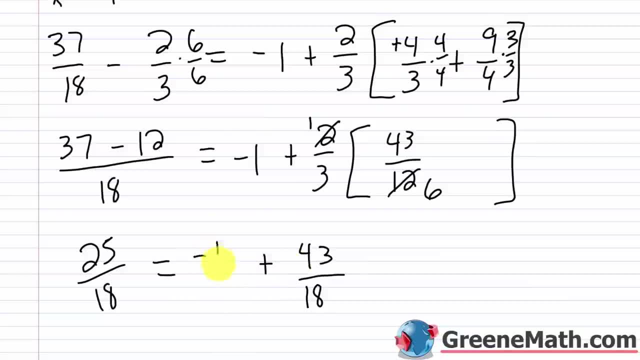 here i'm going to write this negative 1 as negative 18 over 18.. so we just need to think about what is 43 minus 18.. well, that's 25, right? so this becomes 25 18ths. just like on the. 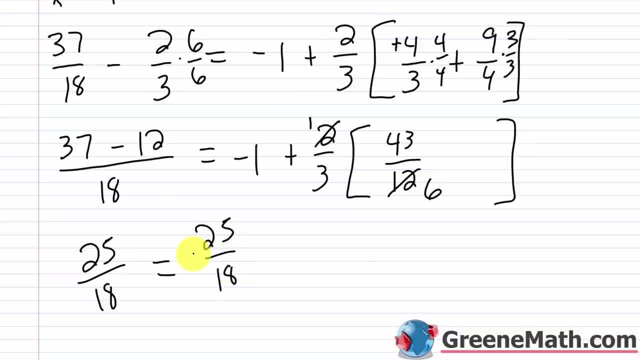 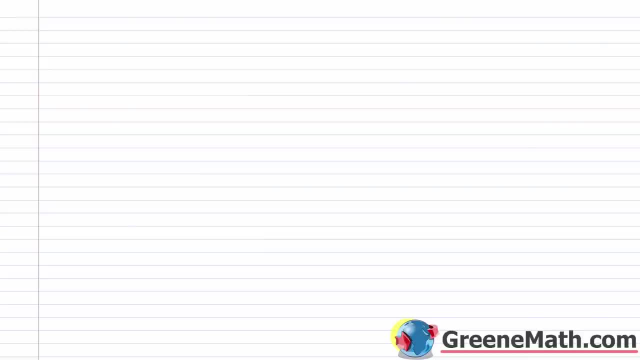 left side of the equation, and so we know that our solution x equals negative 1 is correct. so let's talk a little bit about when your equation has decimals in it. in most cases, you're using calculators on your exams or your homework and working with decimals. when you have a calculator, 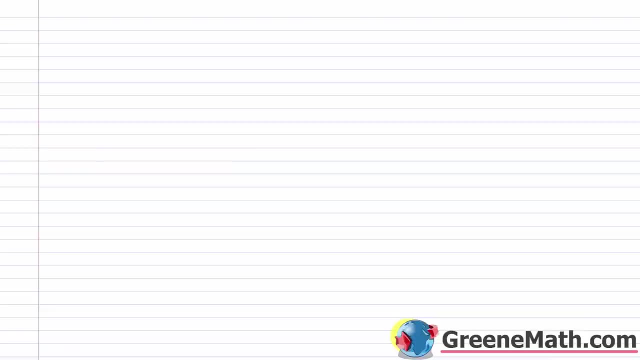 is not any more difficult. so this is just something i'm teaching as a matter of completeness, because you do need to know how to do it, because you might be asked for it on a test, but i don't think it would actually save you any time, especially if you're working with a calculator. 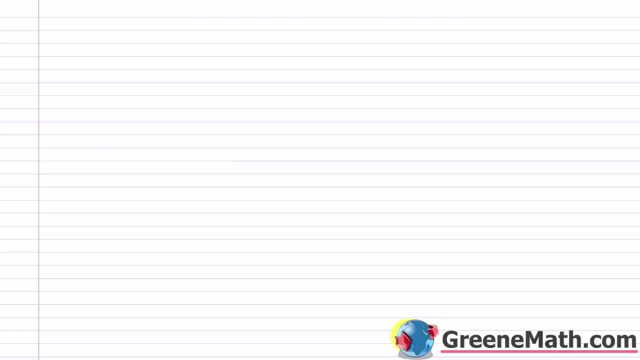 but if you're faced with decimals, i just want you to think back to when we learned that if you multiply by 10, or 10 raised to a whole number that is one or larger, we're going to move our decimal point one place to the right for every. 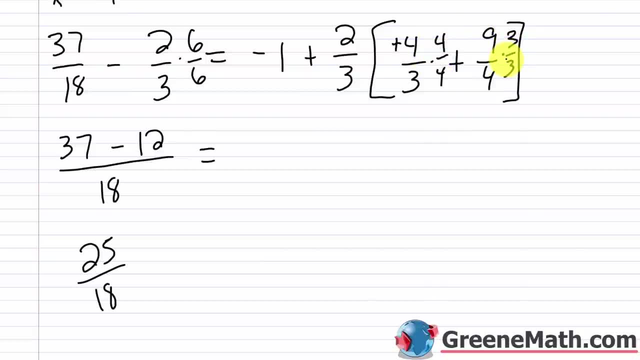 4, I'd multiply this by 3 over 3, and so negative 1 plus 2 thirds times, 4 times 4 is 16 over 12, plus 9 times 3 is 27 over 12, and 16 plus 27 would be 43, so I'd have 43 twelfths. So let me just erase this and write 43 twelfths. So if I'm multiplying here, this is going to cancel with this and give me a 6, and so what I'm going to have is negative 1 plus, I'll have 1 times 43 or 43 over 3 times 6 or 18. So to get a common denominator, here, I'm going to write this negative 1 as negative 18 over 18. So we just need to think about what is 43 minus 18? Well, that's 25, right? So this becomes 25 eighteenths, just like on the 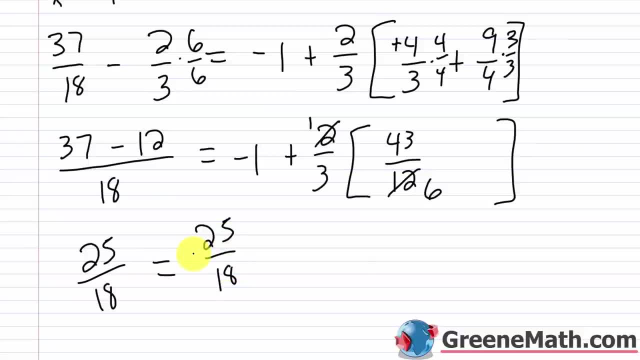 left side of the equation, and so we know that our solution x equals negative 1 is correct. So let's talk a little bit about when your equation has decimals in it. In most cases, you're using 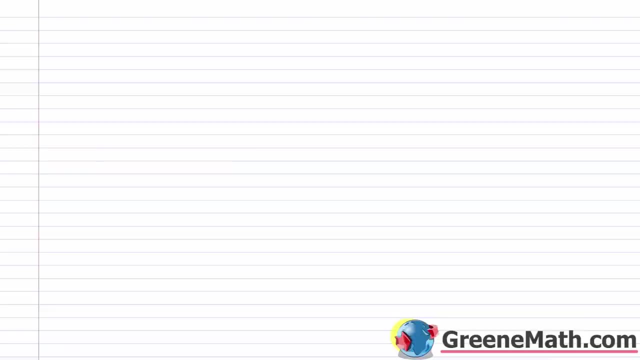 calculators on your exams or your homework, and working with decimals when you have a calculator is not anymore. 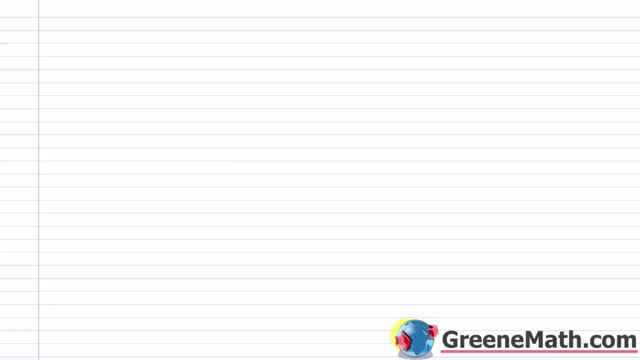 So this is just something I'm teaching as a matter of completeness. You do need to know how to do it because you might be asked for it on a test, but I don't think it would actually save you any time, especially if you're working with a calculator. But if you're faced with decimals, I just want you to think back to when we learned that if you multiply by 10 or 10 raised to a whole number that is one or larger, we're going to move our decimal point one place to the right for every zero in our power of 10. 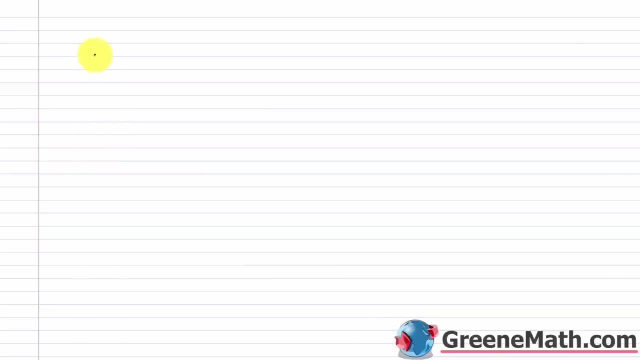 So let's say I have the number 6 and I multiply by 100. Well, I have two zeros in this power of 10, so I take 6, and write a decimal point after 6. You can always write 6 as 6.0, and then I can move the decimal point two places to the right to get my answer because I have two zeros in that power of 10. So this is really 600. We know that six times 100 is 600. 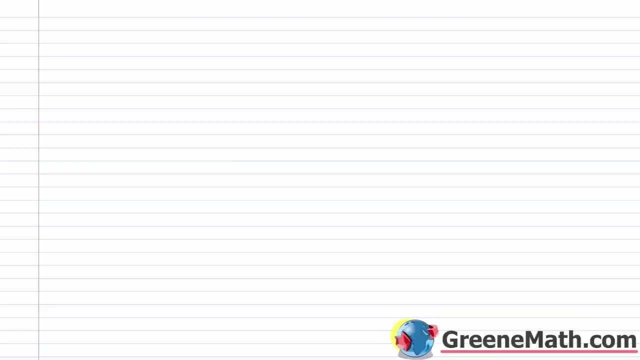 zero in our power of 10.. so, for example, let's say i have the number 6 and i multiply by 100.. well, i have two zeros in this power of 10, and so i take 6. i write a decimal point after 6, because 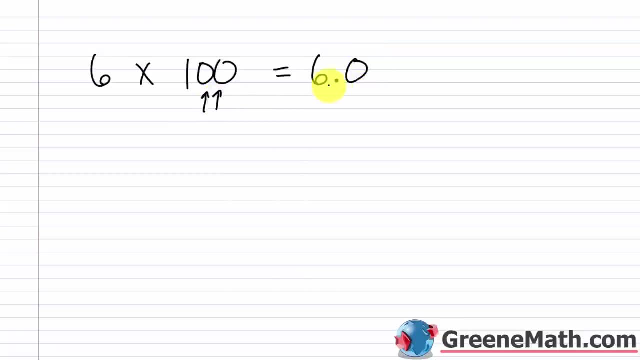 you can always write 6 as 6.0 and then i can move the decimal point two places to the right to get my answer, because i have two zeros in that power of 10.. so this is really 600, right? we know that six times 100 is 600. 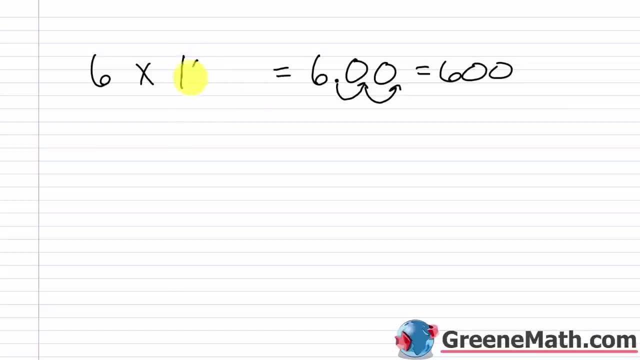 we also could write a hundred as 10 to the second power and kind of the shortcut is the: look at the exponent there and say, okay, i have two places that i'm going to move my decimal point to the right, because if you have a 10 raised to the power of 2, it's going to be a 1, followed by two zeros and one. 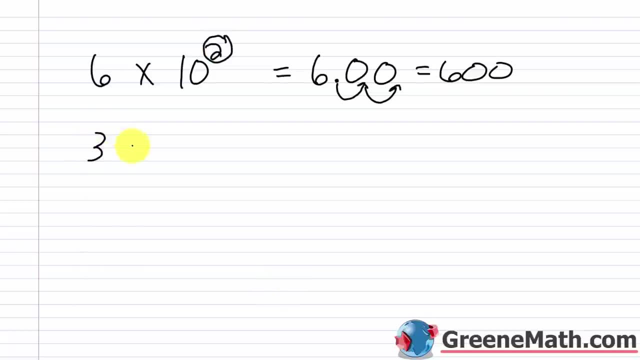 to the fourth, and once you get good at this, you can be very, very quick with these calculations. so let's say i had three times 10 to the fourth power. i see that there's a four here as my exponent. that means that i would have a one followed by four zeros. right, that's what 10 to the fourth is. 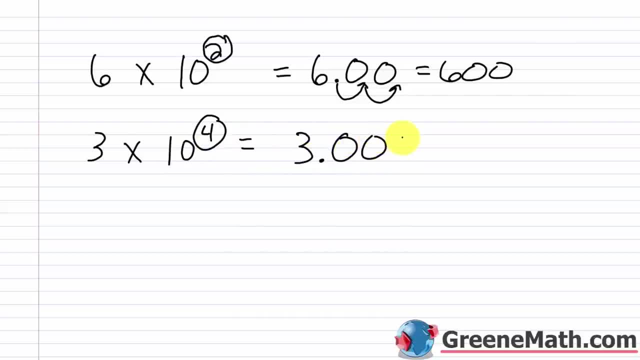 so this would be a three. put my decimal point down and i'm going to move that decimal point four places to the right because there's a four there. so one, two, three, four and i'm going to end up with thirty thousand. right because ten to the fourth power. 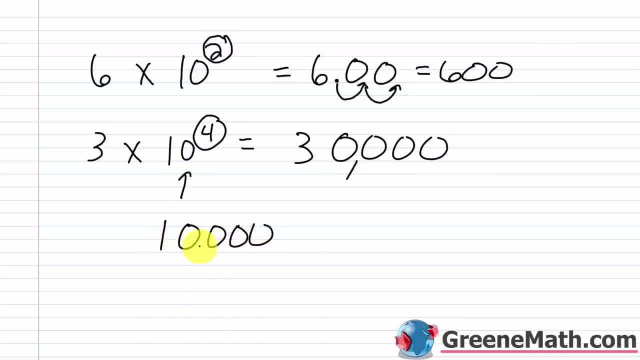 again is a one followed by four zeros. so one, two, three, four or ten thousand, and you can kind of mentally see that three times ten thousand is thirty thousand. it's pretty easy to do so if we do this and we involve, you know kind of some decimals. 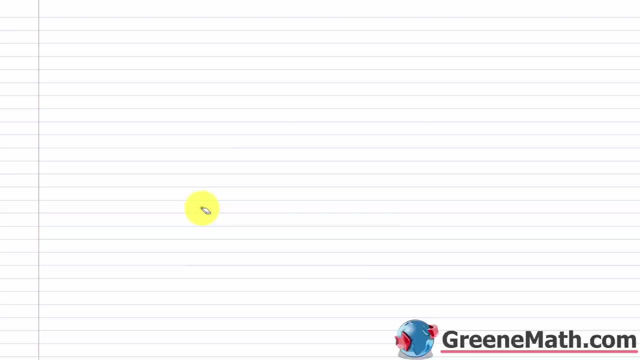 we can kind of use the same principle to clear the decimal. so if we have 6.32- and i want to make this into a whole number- meaning i don't want to see this decimal point anymore- i have one, two decimal places here- all i need to do is multiply it by a number that has a one followed. 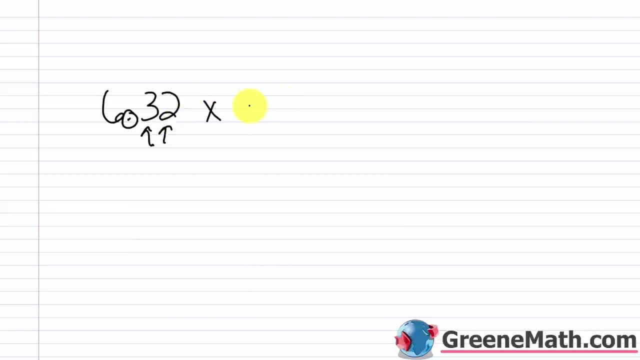 by two zeros, right. so i'd multiply it by a hundred, or ten squared times a hundred. so this would be equal to 632, right, because this would go one, two places to the right. so, essentially, what's going to end up happening is we're going to look at our equation and we're going to see the largest number. 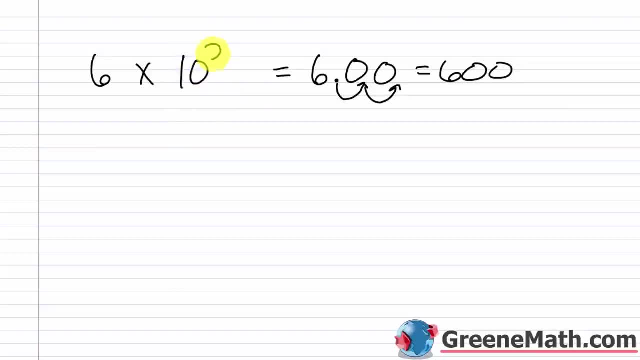 write 100 as 10 to the second power. And kind of the shortcut is the look at the exponent there and say, okay, I have two places that I'm going to move my decimal point to the right. Because if you have a 10 raised to the power of two, it's going to be a one followed by two zeros. And once you get good at this, you can be very, very quick with these calculations. So let's say I had three times 10 to the fourth power. I see that there's a four here as my exponent. That means that I would have a one followed by four zeros, right? That's what 10 to the fourth is. So this would be a three, put my decimal point down, and I'm going to move that decimal point four places to the right because there's a four there. So one, two, three, four, and I'm going to end up with 30,000. 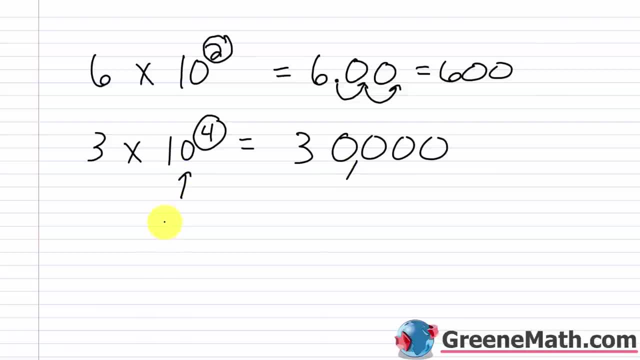 Because 10 to the fourth power, 10 to the fourth power, again, is a one followed by four zeros. So one, two, three, four, or 10,000. And you can kind of mentally see that three times 10,000 is 30,000. It's pretty easy to do. So if we do that, we're going to have a one followed by four zeros. So that's what 10 to the fourth power is. 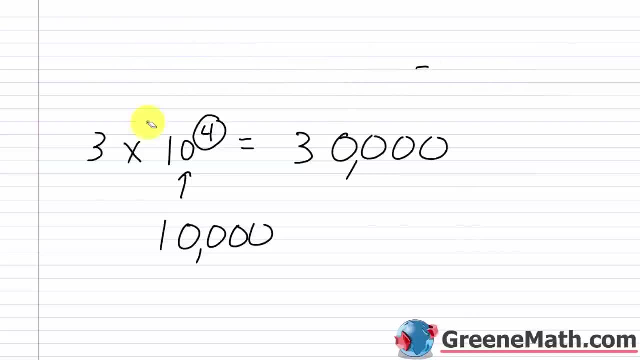 And if we do this and we involve, you know, kind of some decimals, we can kind of use the same principle to clear the decimals. So if we have 6.32, 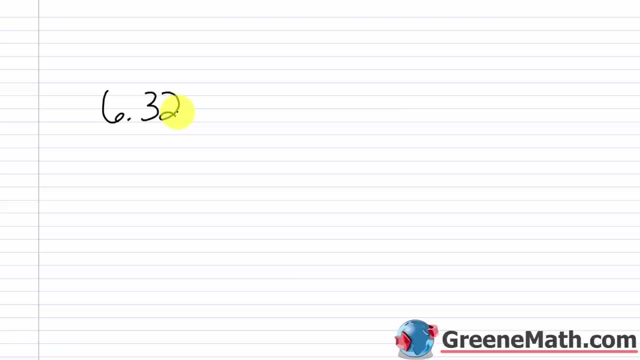 and I want to make this into a whole number, meaning I don't want to see this decimal point anymore, I have one, two decimal places here. All I need to do is multiply it by a number that has a one followed by two zeros, right? So I'd multiply it by 100 or 10 squared. 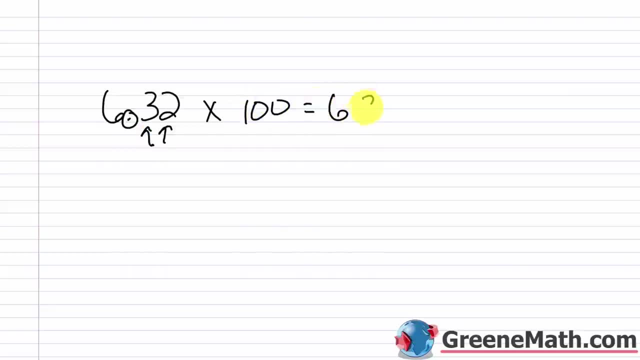 So times 100. So this would be equal to 632, right? Because this would go one, two places to the right. So essentially, what's going to end up happening is we're going to look at our equation, and we're going to see the largest number of decimal places between everything involved. So we're then going to multiply both sides of the equation by a power of 10 that will clear that decimal. So you want to clear the largest number of decimal places. So if the largest number of decimal places you have is three, then you're going to multiply by 1000, right? It's a power of 10 that has a one followed by three zeros. And if you clear the one that has the largest number of decimal places, you're going to clear all. All right, so let's take a look at 20.01 equals negative 6.7 minus 10.7 n minus 8.6. 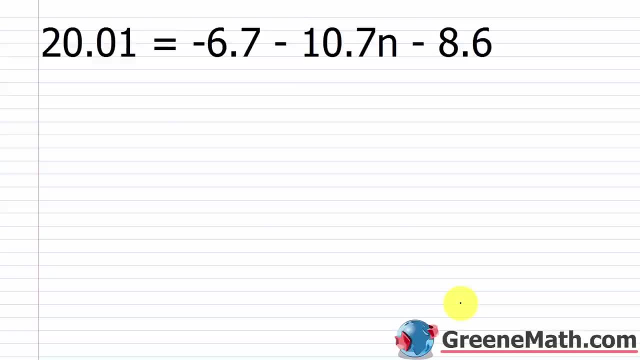 of decimal places between everything involved. so we're then going to multiply both sides of the equation by a power of two. so we're going to multiply both sides of the equation by a power of ten. that will clear that decimal. so you want to clear the largest number of decimal places. so 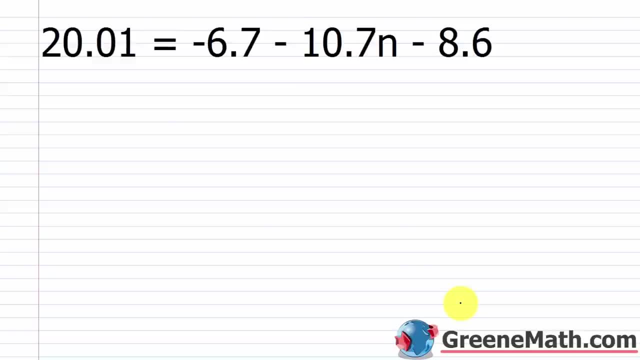 if the largest number of decimal places you have is three, then you're going to multiply by a thousand, right? it's a power of ten that has a one followed by three zeros, and if you clear the one that has the largest number of decimal places, you're going to clear all of them. all right, so let's take a. 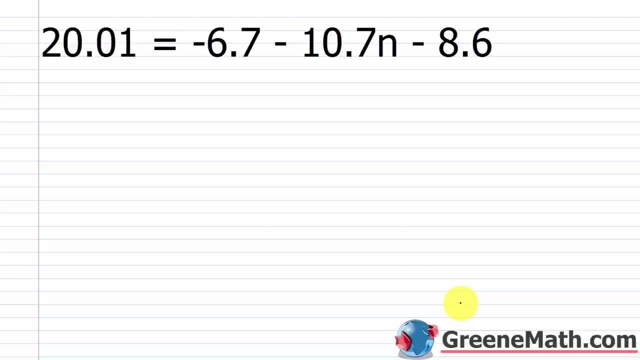 look at: 20.01 equals negative 6.7 minus 10.7. n minus 8.6. i'm going to look through this equation and you're going to see that i have one, two decimal places here. i have one decimal place here. 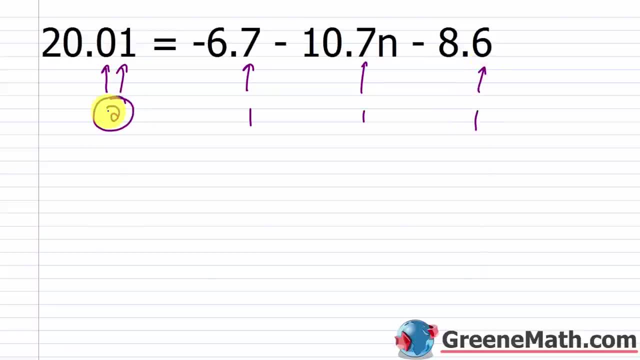 one here and one here, so the largest number of decimal places between any of these numbers involved would be two. now, in order to clear the equation of decimals, i need to multiply by a power of ten. that will allow me to move all the decimal points in the equation two places to the right. 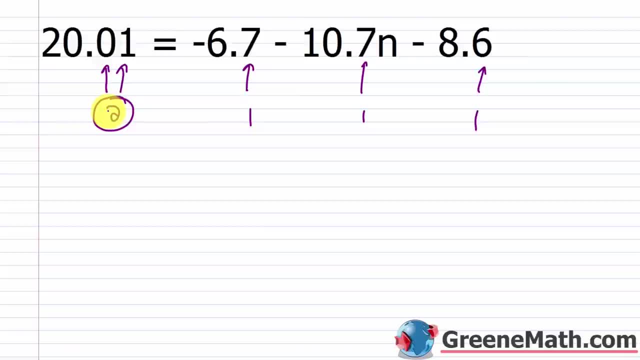 so to do that, you're going to multiply by a hundred. okay, just think about: okay, i need two zeros in the equation, so i'm going to multiply by a hundred. so i'm going to multiply by a hundred. so that's 10 squared or 100.. 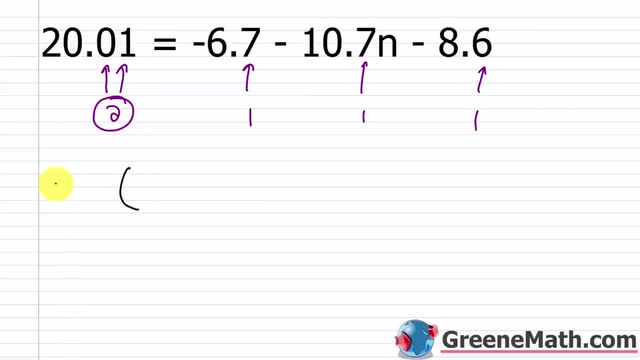 so again, i'm going to use parentheses or brackets to put 100 outside, 20.01 equals, and i have a 100 outside of here too. negative: 6.7 minus 10.7, n minus 8.6. very, very easy, now we're. 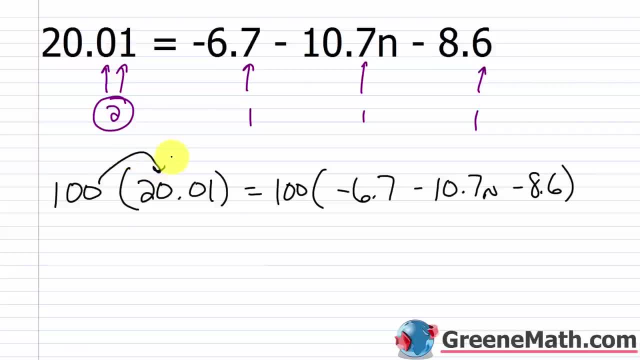 just going to use our distributive property. so 100 times 20.01, again move your decimal point two places to the right. so this would be a decimal point two places to the right. so this would be a two thousand one. this is equal to, over here, 100 times negative 6.7, you'll have negative, you'll have. 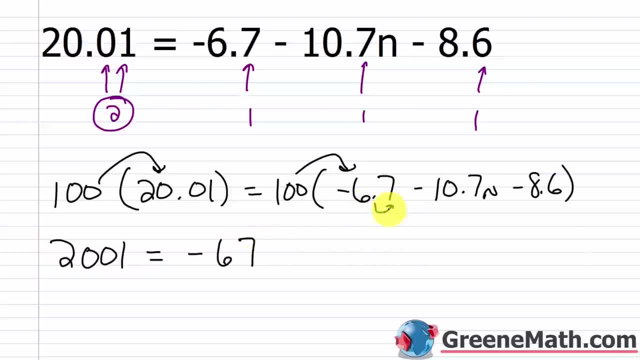 six. this is going to go one. so i'll have a seven, and then one more place to the right, and so a zero, so negative 670, and then minus. here we have 10.7 n, so i'm going to have 10. this is going to go one. 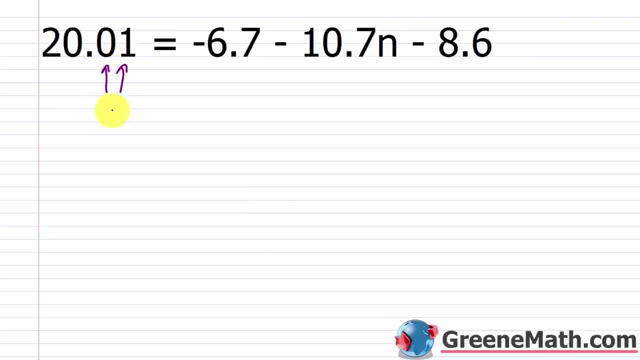 I'm going to look through this equation. I have one, two decimal places here. I have one decimal place here, one here, and one here. So the largest number, of decimal places between any of these numbers involved would be two. Now, in order to clear the equation of decimals, I need to multiply by a power of 10 that will allow me to move all the decimal points in the equation two places to the right. So to do that, you're going to multiply by 100. Okay, just think about, okay, I need two zeros in the power of 10. So that's 10 squared or 100. 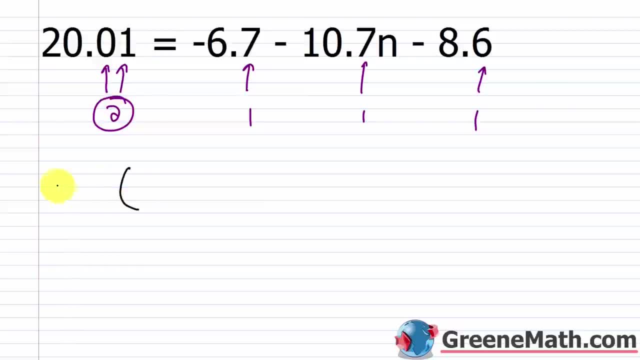 So again, I'm going to use parentheses or brackets to put 100, outside 20.01 equals, and I have a 100 outside of here too, 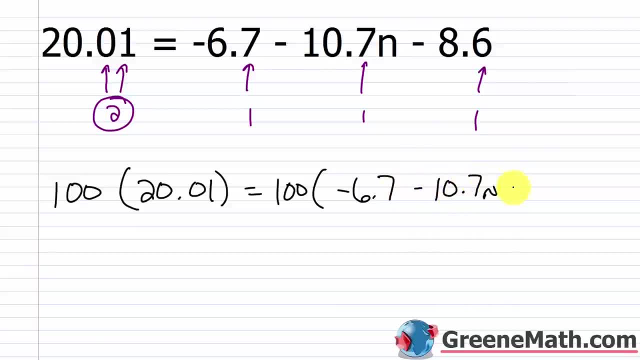 negative 6.7 minus 10.7 n minus 8.6. Very, very easy. Now we're just going to use our distributive property. So 100 times 20.01, again, move your decimal point two places to the right. 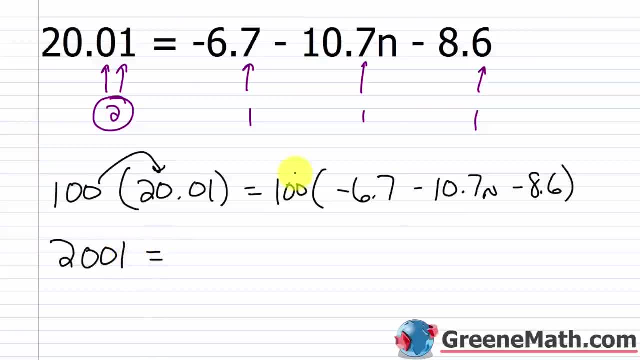 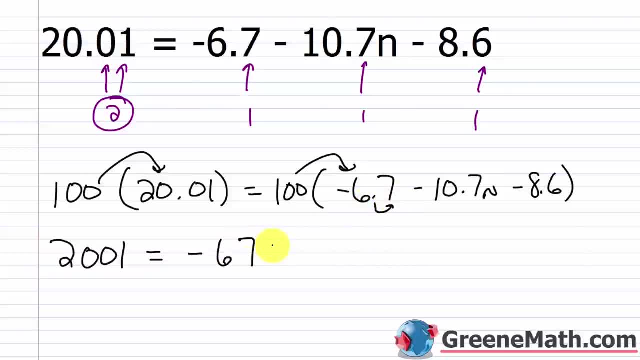 you'll have 6. This is going to go 1. So I'll have a 7 and then one more place to the right. 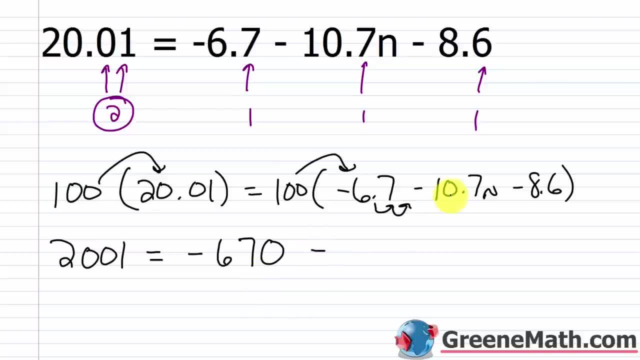 And so a 0. So negative 670. And then minus, here we have 10.7 n. So I'm going to have 10. 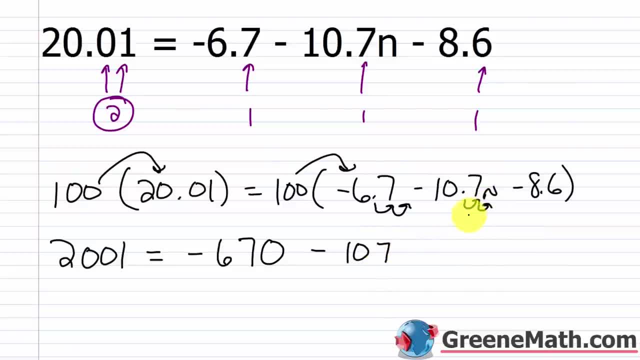 This is going to go one place to the right. That's going to be a 7. One more place to the right. 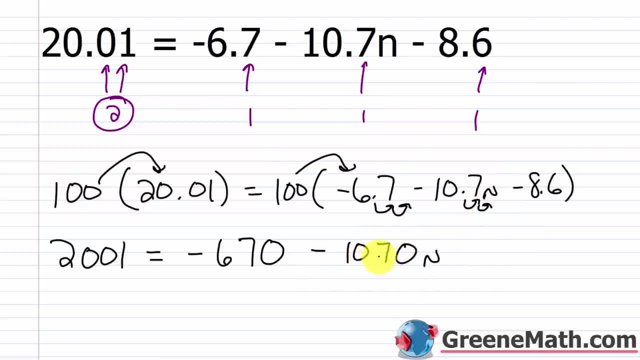 That's going to be a 0. And then my n. So that's minus 1070 n. And then minus, here we have 8.6. 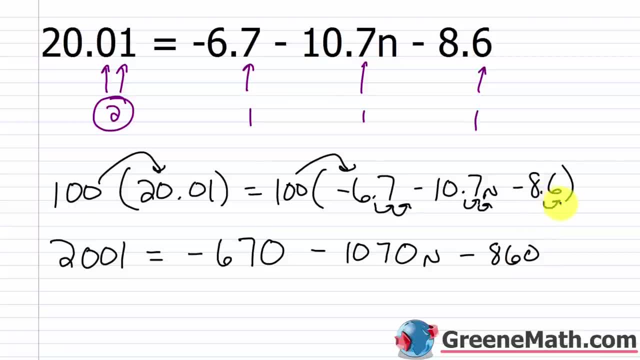 So that's going to be 860, right? This is going to go one, two places to the right. So it's going to go right here and then right there. So we have a transformed equation now that doesn't have 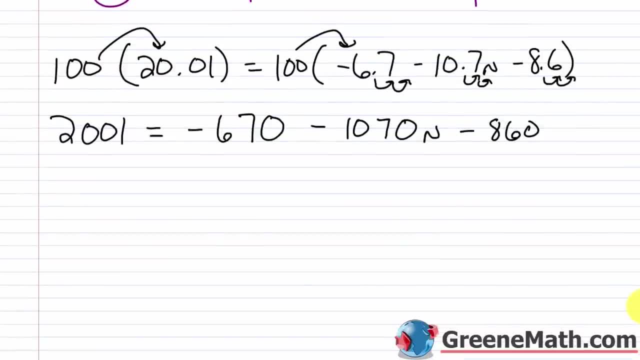 any decimals involved. And again, you just go through after you have this and do your regular procedure. So I would combine like terms here on the right. Negative 670 minus 860 is negative 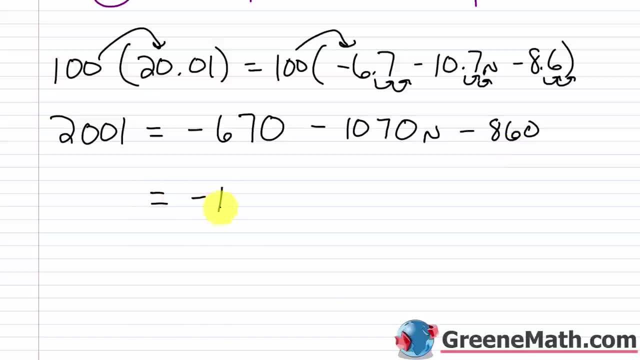 1,530. So this will be negative 1,070 n and then minus 1,530. And this is equal to over here on the left, we have 2001. So I still want to isolate my variable. 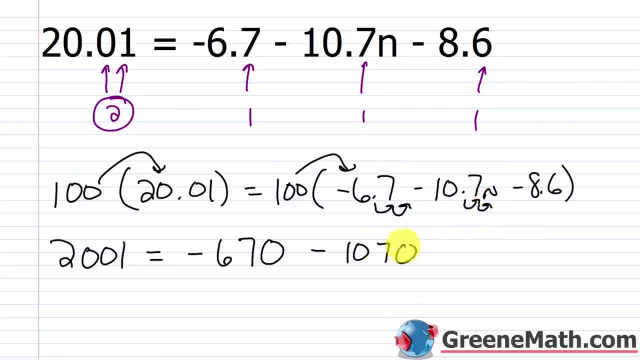 place to the right, that's going to be a seven. one more place to the right, that's going to be a zero, and then my n, So that's minus 1,070n, And then minus, here we have 8.6.. So that's going to be. 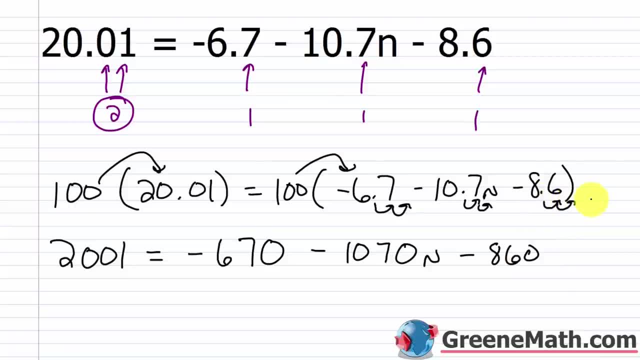 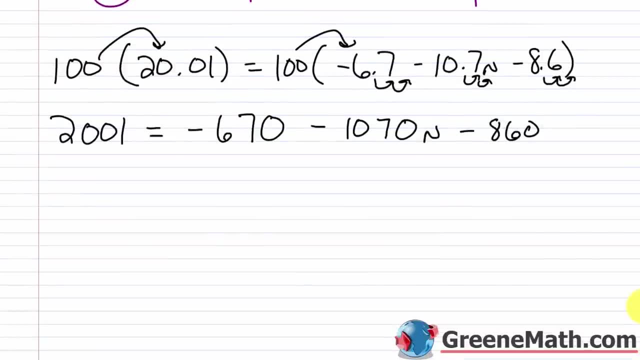 860,. right, This is going to go one, two places to the right, So it's going to go right here and then right there. So we have a transformed equation now that doesn't have any decimals involved And again, you just go through after you have this and do your regular procedure. So 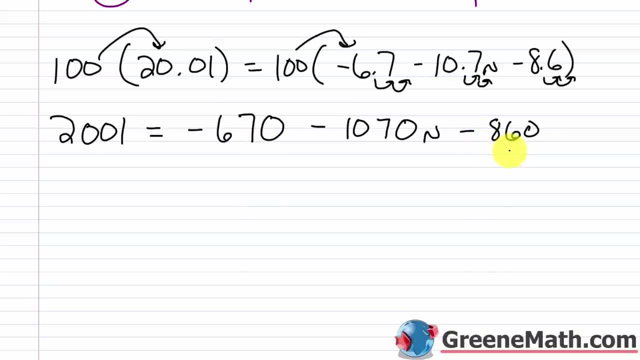 I would combine like terms here on the right: Negative 670 minus 860 is negative 1,530. So this will be negative 1,070n and then minus 1,530. And this is equal to over here on the left. 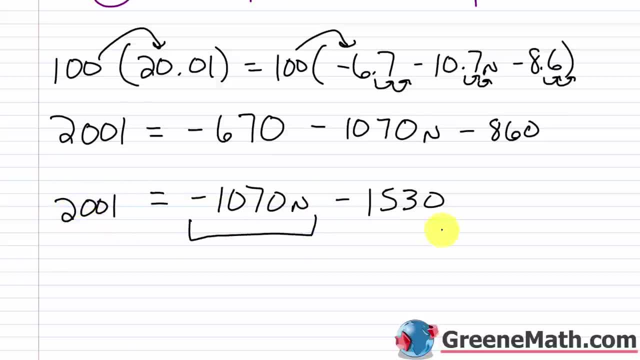 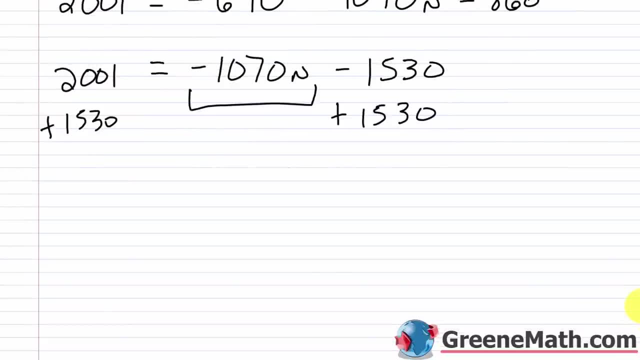 we have 2,001.. So I still want to isolate my variable term And to do that, I'm going to add 1,530 to both sides of the equation, And so 2,001 plus 1,530 is 3,531. And this equals: 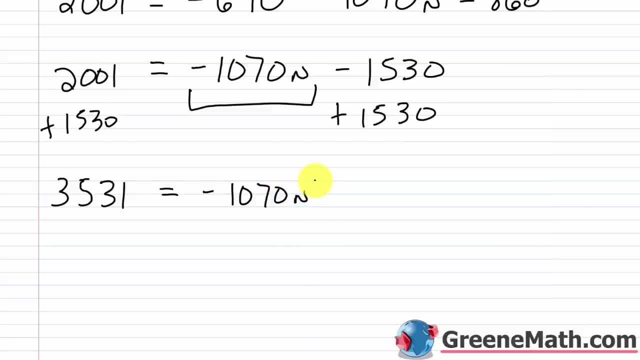 negative 1,070.. All right, now to get n by itself. I just divide both sides of the equation by the coefficient. So divide by negative 1,070,, divide by negative 1,070.. And this will cancel with this And then 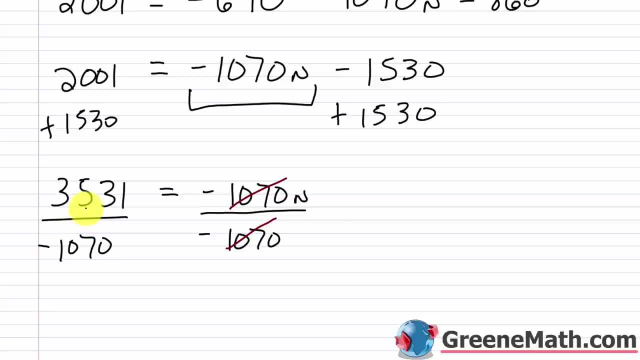 3,531 divided by negative 1,070 is going to give me negative 3.3. So I get negative 3.3 equals n. Now notice how I wrote it like that, versus as a fraction. You can do either, Because we're working with decimals. I chose to write this as a decimal. 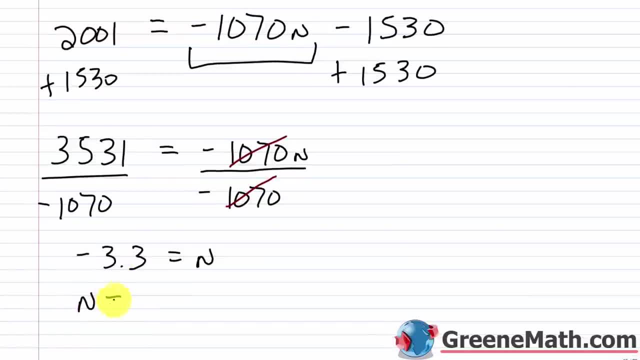 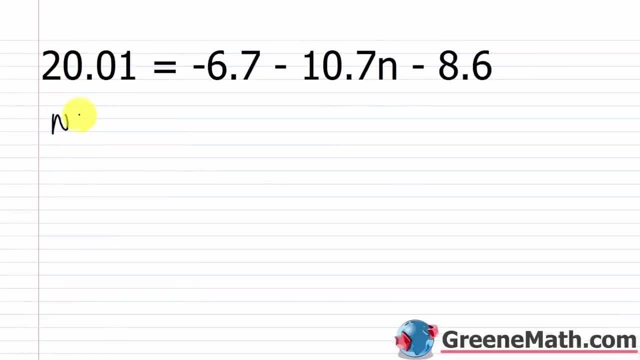 You can do either one, It does not matter. So I'm going to rewrite this as n equals negative 3.3.. And we're going to go back up to the top and check it. Okay, so we're going to have n equals. 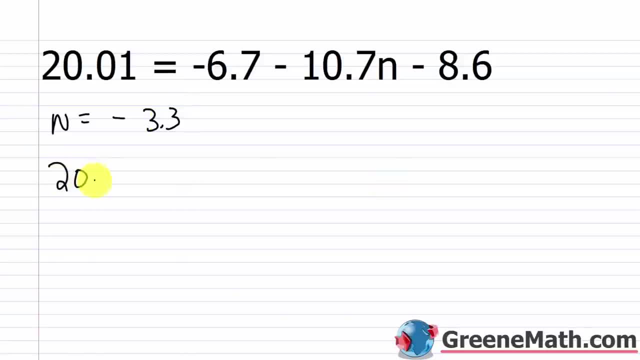 negative 3.3 here. So we're going to have: 20.01 is equal to negative 6.7 minus 10.7 times. again, negative 3.3 minus 8.7.. Okay, so over here on the left, 20.01 is not going to change. Don't need to do anything there. 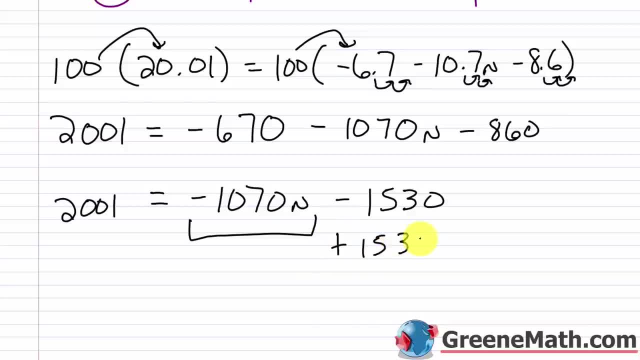 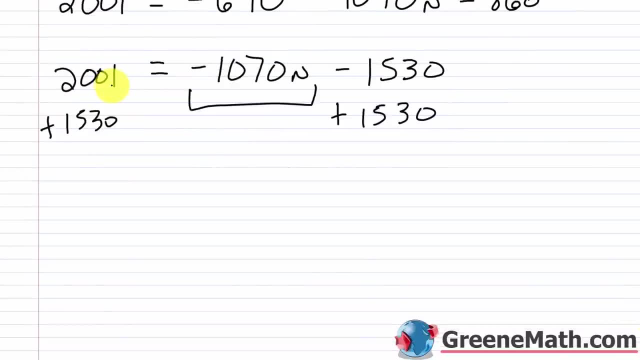 And to do that, I'm going to add 1,530 to both sides of the equation. And so 2001 plus 1,530 is 3,531. And this equals negative 1,070 n. All right. Now to get n by itself, I just divide both sides of the equation by the coefficient. So divide by negative 1,070, divide by negative 1,070. This will cancel with this. And then 3,531 divided by negative 1,070 is going to give me negative 3.3. So I get negative 3.3 equals n. Now notice how I wrote it like that versus as a fraction. You can do either. Because we're working with decimals, I chose to write this as a decimal. You can do either one. It does not matter. So I'm going to rewrite this as n equals negative 3.3. 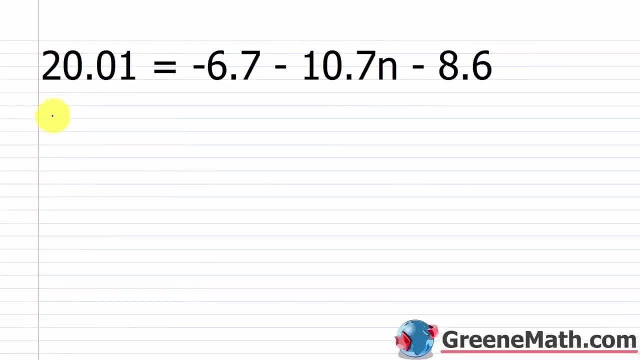 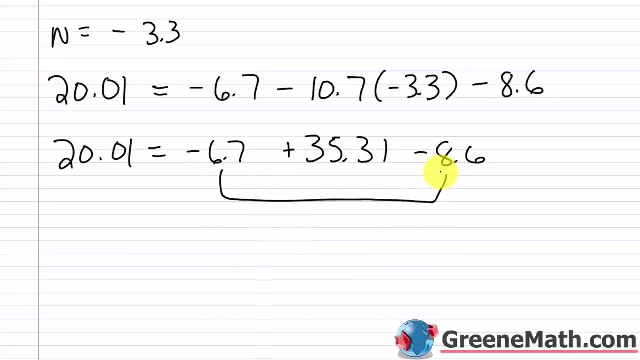 And we're going to go back up to the top and check it. Okay. So we're going to have n equals negative 3.3 here. So we're going to have 20.01 is equal to negative 6.7 minus 10.7 times, again, negative 3.3 minus 8.6. Okay. So over here on the left, 20.01 is not going to change. Don't need to do anything there. On the right, I need to do my multiplication first. What is negative 10.7 times negative 3.3? It's going to give me 35.31. 35.31. Okay. So now I have negative 6.7 plus 35.31 minus 8.6. So I'm going to add my numbers with like signs first. What is negative 6.7 minus 8.6? That's going to be negative 15.3. So I'm going to write this as 20.01 equals... Negative 15.3 plus 35.31. And now we just need to add over here. What is negative 15.3 plus 35.31? That's going to give me 20.01. So 20.01 equals 20.01. Same number on the left and the right. So n equals negative 3.3 is the correct solution. All right. Let's take a look at another one. 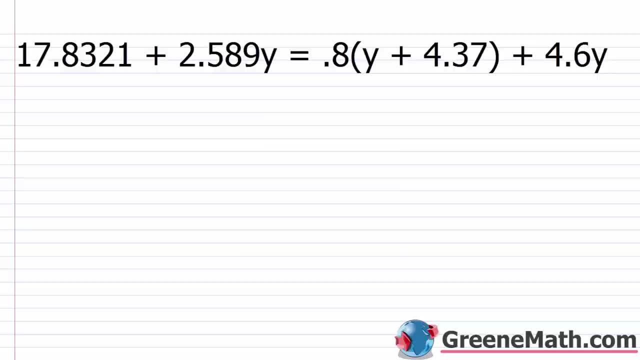 We have 17.8321 plus 2.589y equals 0.8 times the quantity y plus... 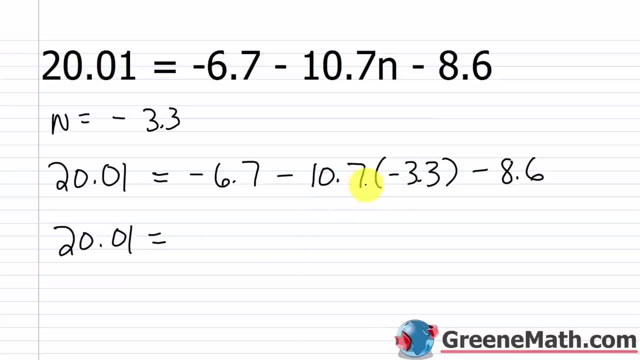 On the right. I need to do my multiplication first. What is negative? 10.7 times negative 3.3? It's going to give me 35.31.. 35.31.. Okay, so now I have negative 6.7 plus 35.31 minus 8.6.. 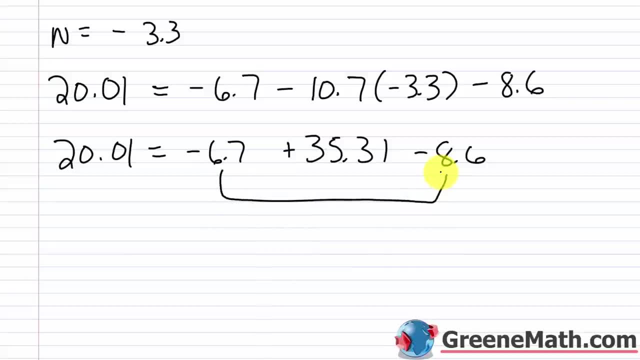 So I'm going to add my numbers with 1.6.. So I'm going to add my numbers with 1.6.. So I'm going to like signs first. What is negative? 6.7 minus 8.6? That's going to be negative 15.3.. 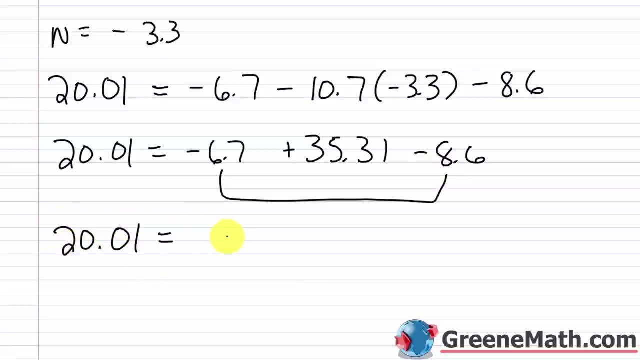 So I'm going to write this as: 20.01 equals negative 15.3 plus 35.31.. And now we just need to add over here What is negative: 15.3 plus 35.31? That's going to give me 20.01.. So 20.01 equals 20.01.. Same number on the left and the right. 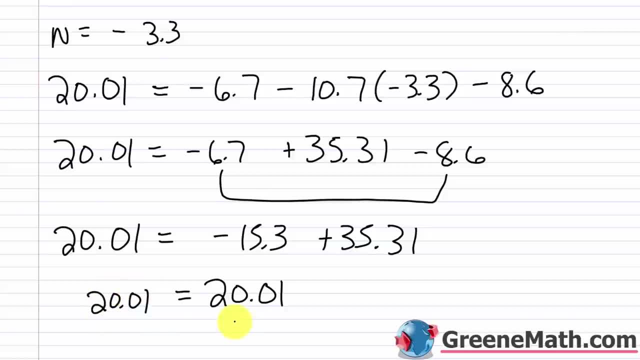 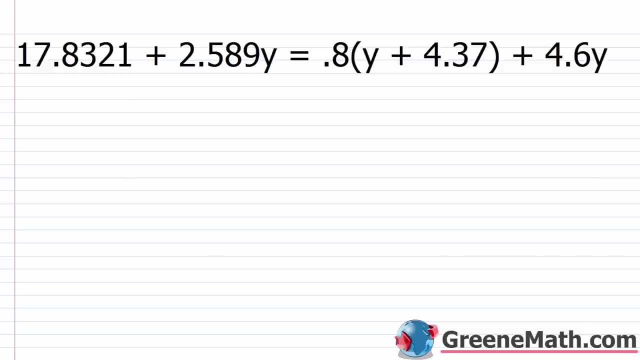 So n equals negative 3.3.. 3.3 is the correct solution. All right, let's take a look at another one. We have 17.8321 plus 2.589Y equals 0.8 times the quantity Y plus 4.37 plus 4.6Y. 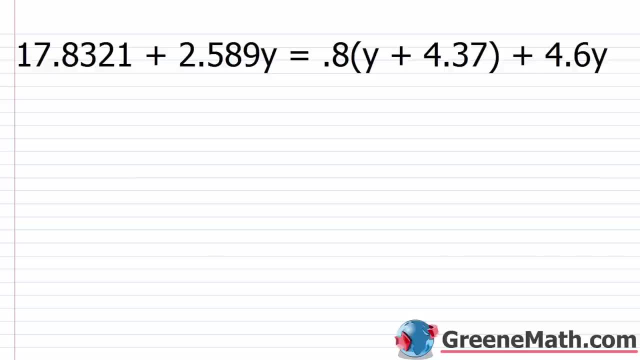 Now, just like we saw with fractions, when you're trying to clear decimals you've got to use your distributive property first if you have decimals inside the parentheses. So 17.8321 plus 2.589Y equals, distribute this inside here. 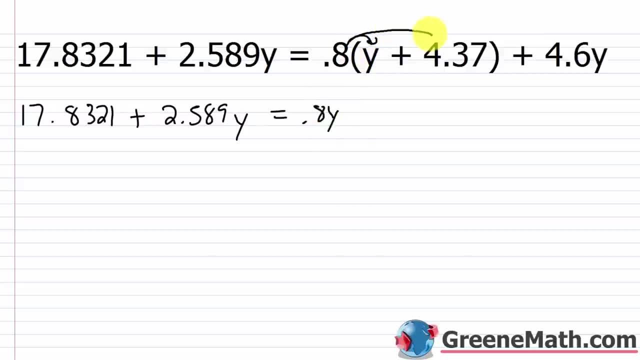 so 0.8 times Y is 0.8Y. and then distribute this inside here: so plus So 0.8 times 4.37 is 3.496.. So 3.496 plus 4.6Y. 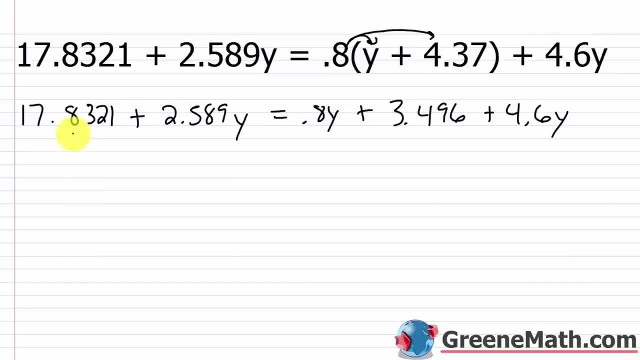 So now I'm gonna look to see what number has the highest number of decimal places. I have one, two, three, four here. I have one, two, three here, I have one here, one, two, three here, And I have one here. 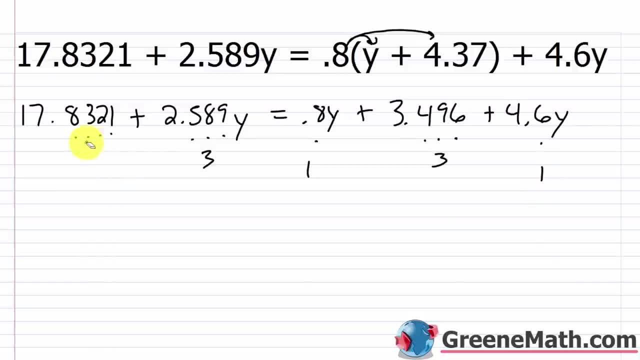 So the highest number of decimal places is four. So that means I need to multiply by a number that has a one followed by four zeros. So I'm gonna multiply both sides of this equation by a one followed by one, two, three, four zeros. 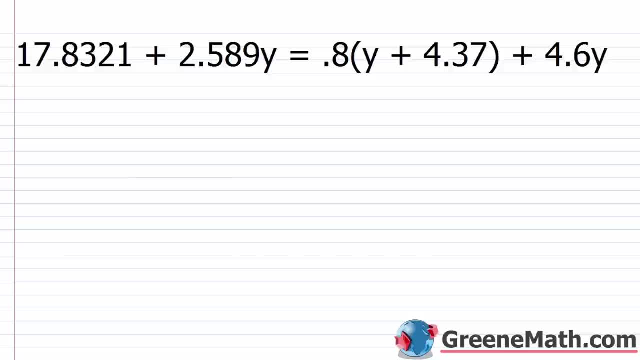 4.37 plus 4.6y. Now, just like we saw with fractions, when you're trying to clear decimals, you've got to use your distributive property first if you have decimals inside the parentheses. So 17.8321 plus 2.589y equals... Distribute this inside here. So 0.8 times y is 0.8y. And then distribute this inside here. So plus... So 0.8 times 4.37. So 0.8 times 4.37 is 3.496. So 3.496 plus 4.6y. So now I'm going to look to see what number has the highest number of decimal places. I have 1, 2, 3, 4 here. I have 1, 2, 3 here. I have 1 here. 1, 2, 3 here. And I have 1 here. So the highest number of decimal places is 4. So that means I need to multiply by a number that has a 1 followed by four zeros. So I'm going to multiply by a number that has a 1 followed by four zeros. 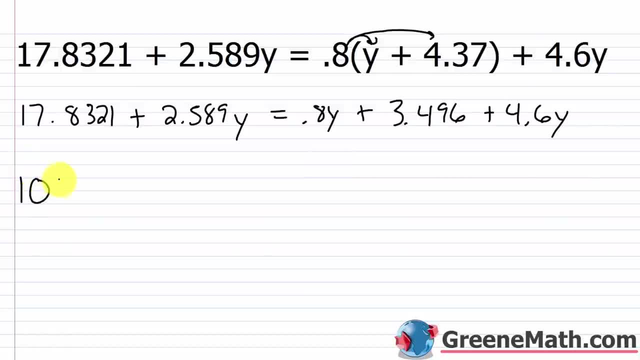 I'm going to multiply both sides of this equation by a 1 followed by 1, 2, 3, 4 zeros for the number 10,000. So I'm going to have 10,000 times 17.8321 plus 2.589y. And again, make sure to put this inside of parentheses. You're really multiplying 10,000 by each of these numbers. You can't make 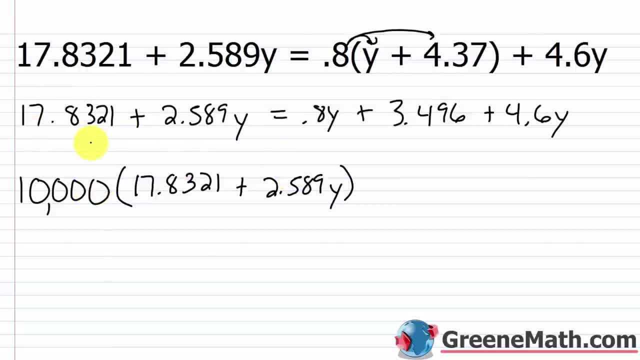 the mistake of just multiplying it by 17.8321. It's also got to be multiplied by 2.589y. 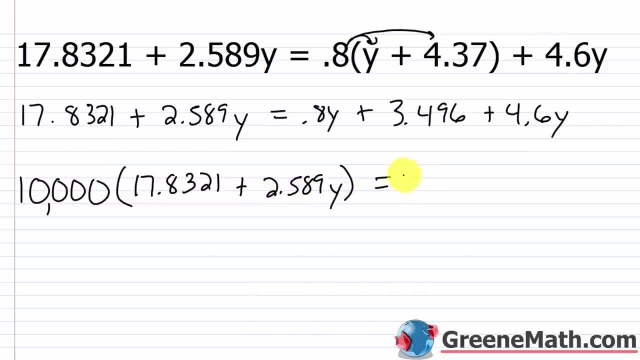 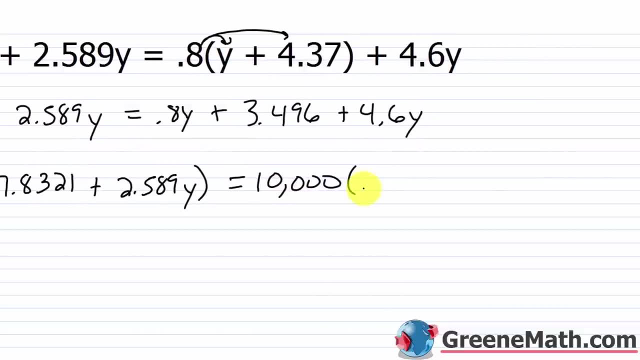 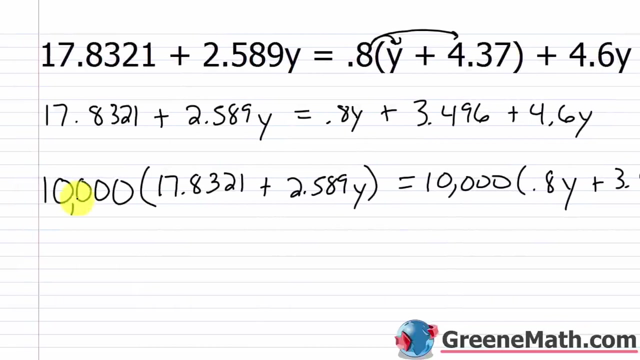 Okay. So over here, I'm going to have 10,000 also multiplied by, and I'm going to need to put this off the screen for a minute. So we'll have 0.8y plus 3.496 plus 4.6y. Again, inside of parentheses. Okay. So starting over here on the left, if I multiply 10,000 times 17.8321, it's 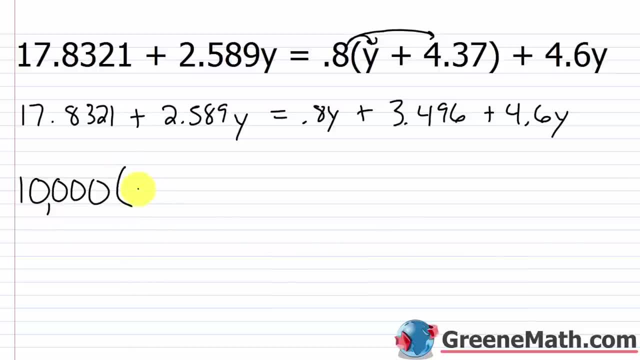 for the number 10,000.. So I'm gonna have 10,000 times 17.8321.. Plus 2.589Y, And again make sure to put this inside of parentheses. You're really multiplying 10,000 by each of these numbers. 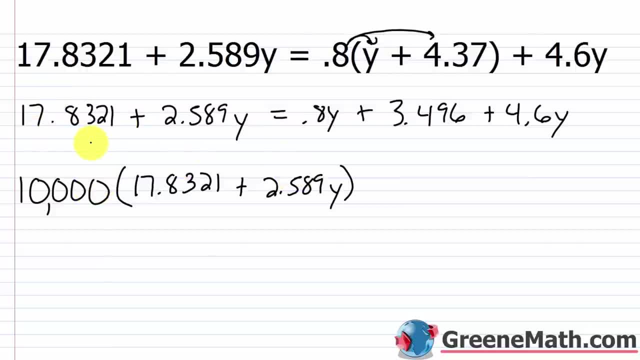 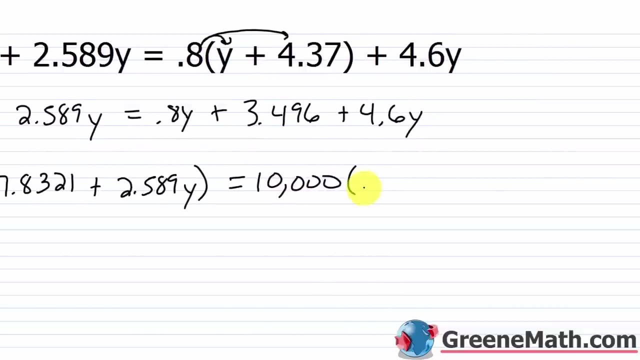 You can't make the mistake of just multiplying it by 17.8321.. It's also gotta be multiplied by 2.589Y as well, Okay. so over here I'm gonna have 10,000 also multiplied by, and I'm gonna need to put this off the screen for a minute. 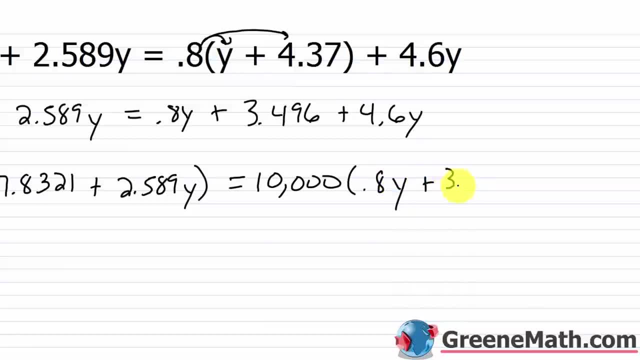 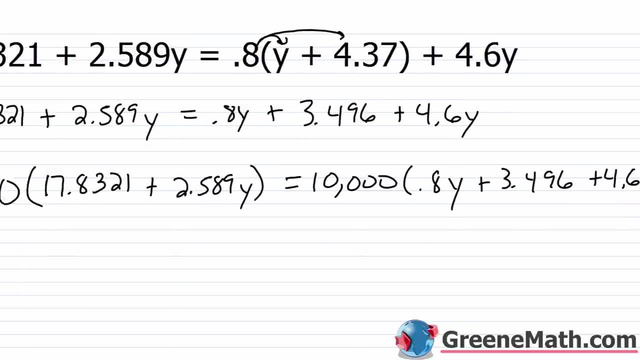 So we'll have 0.8Y Plus 3.496.. Plus 4.6Y, Again inside of parentheses. Okay, So, starting over here on the left, if I multiply 10,000 times 17.8321,. 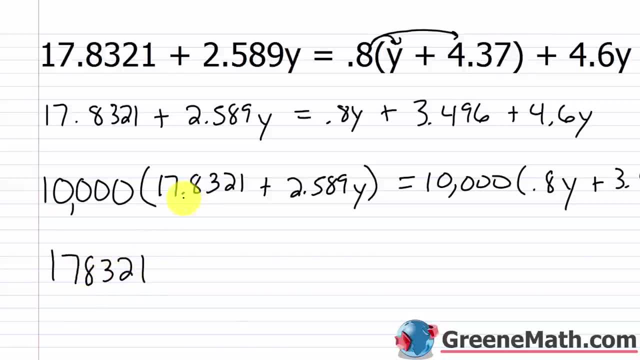 it's gonna be 178321.. Right, this will go four places to the right, And so I end up with 178321.. So then, plus now, if I multiply 10,000 by 2.589Y, I'm basically gonna have. okay, I'm gonna have. 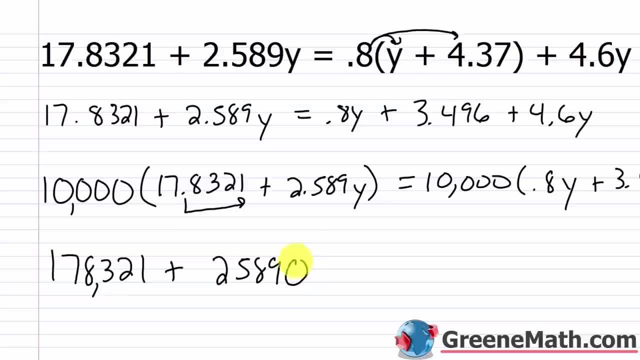 two, five, eight, nine and then a zero at the end. again, this goes four places to the right, and so it would pass the nine and then go one more right. so that's why i have the zero. here we go one, two, three, four places to the right, so that ends up giving me 25, 890, and then times the. 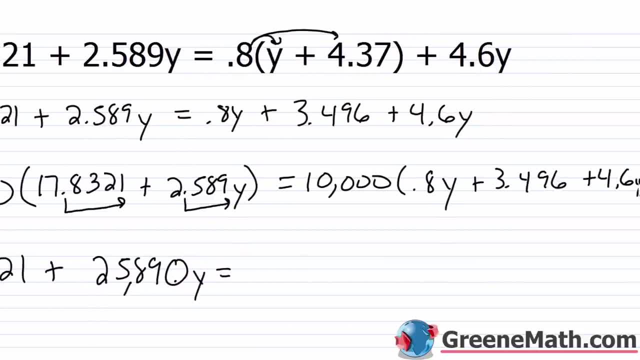 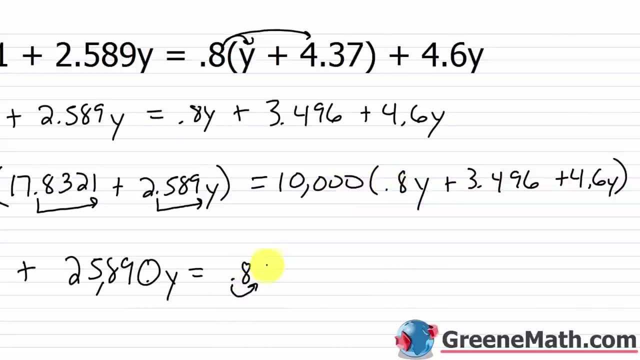 variable y and then over here on the right, i have 10 000 times 0.8 y, so i have 0.8, and this goes four places to the right. it's going to go one, two, three, four, so that's going to be 8 000 then 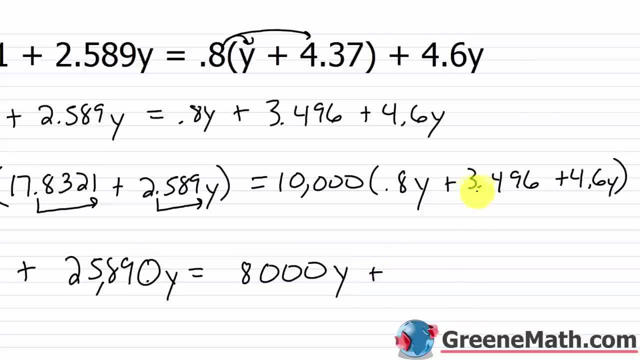 again times the variable y, then plus over. here i have 3.496. so this is going to go four places to the right. so it's going to pass the six by one more place. so i'm going to need to write three, four, nine, six, zero, right? this is going to go one, two, three, four places to the right and then plus. 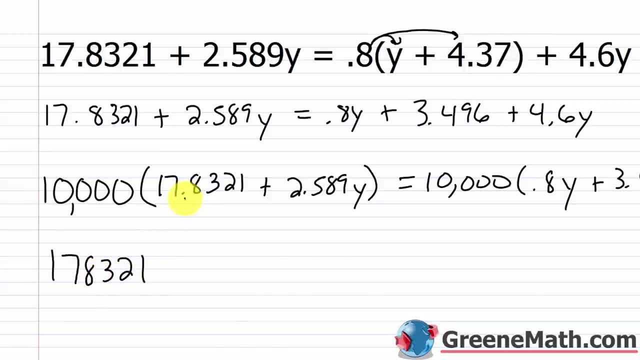 going to be 1, 7, 8, 3, 2, 1, right? This will go four places to the right. And so I end up with 178,321. So then plus, now if I multiply 10,000 by 2.589y, I'm basically going to have 2, 5, 8, 9, and then a zero at the end. Again, this goes four places to the right. And so it would pass the nine and then go one more, right? So that's why I have the zero here. It would go 1, 2, 3, 4. 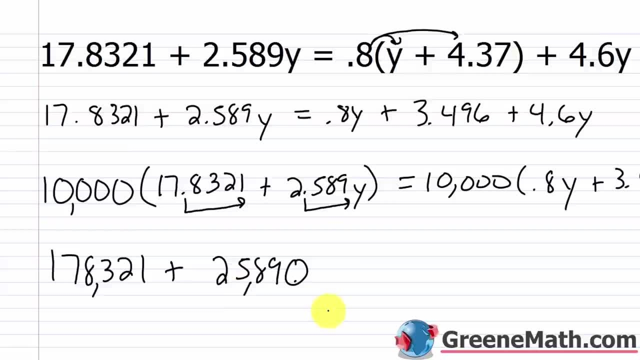 Four places to the right. So that ends up giving me 25,890 and then times the variable y. 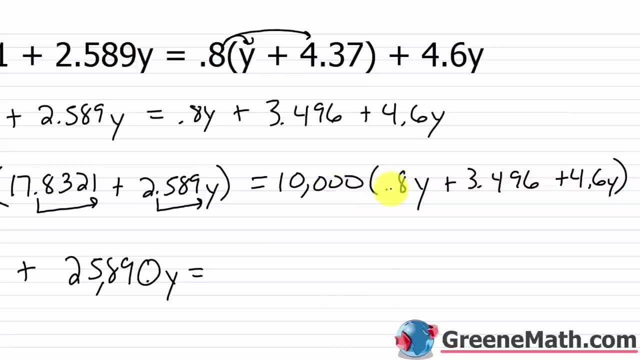 And then over here on the right, I have 10,000 times 0.8y. So I have 0.8 and this goes four places to the right. It's going to go 1, 2, 3, 4. So that's going to be 8,000. Then again, 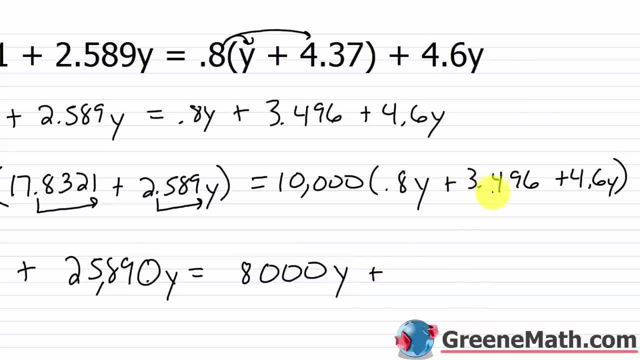 times the variable y. Then plus over here, I have 3.496. So this is going to go four places to the right. So it's going to pass the six by one more. So I'm going to need to write 3, 4, 9, 6, 0, right? This is going to go 1, 2, 3, 4 places to the right. And then plus, we have 4.6y. So 10,000 times 4.6, we think about 46 here. And I'm going 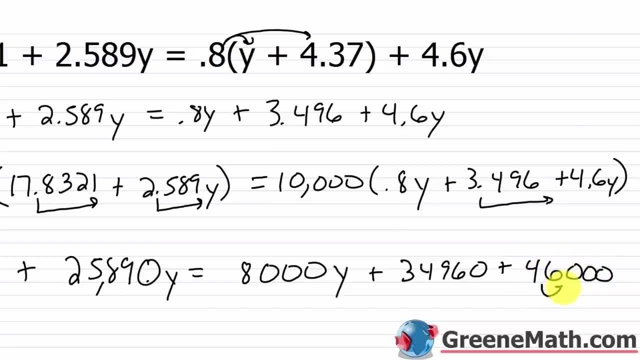 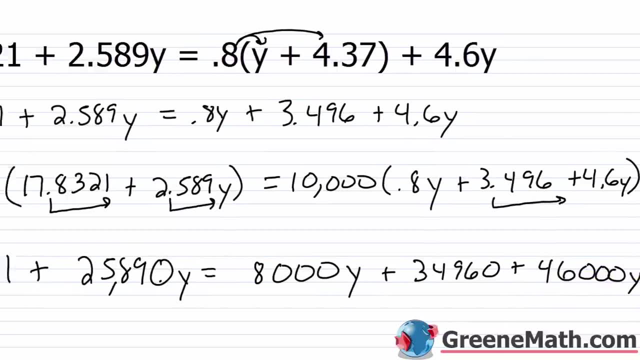 to need to put three more zeros. 1, 2, 3. This is going to go 1, 2, 3, 4 places to the right. And then don't forget the y. And then we have our transformed equation. 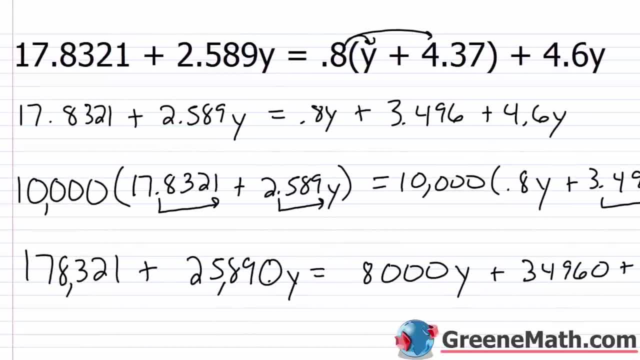 Unfortunately, it's so big, it doesn't fit on the screen. But we go through the same process. 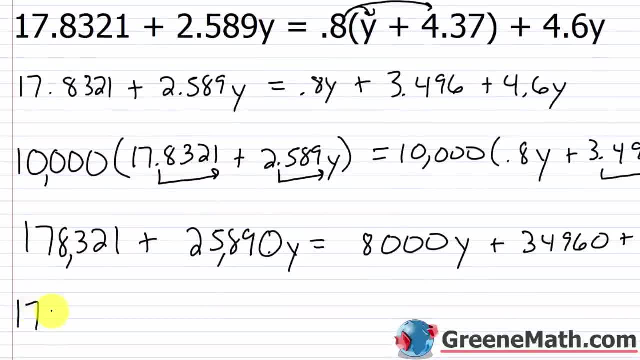 On the left, I can't simplify any more. So I'm just going to write 178,321 plus 25,890y. 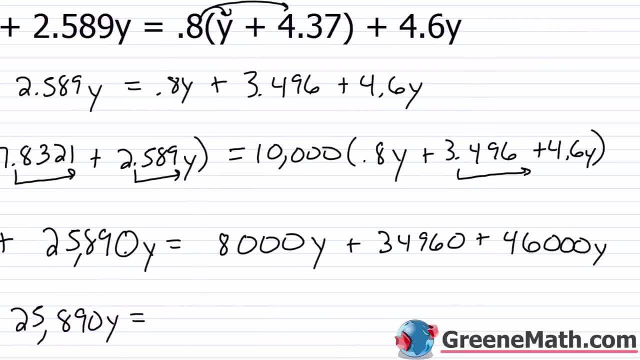 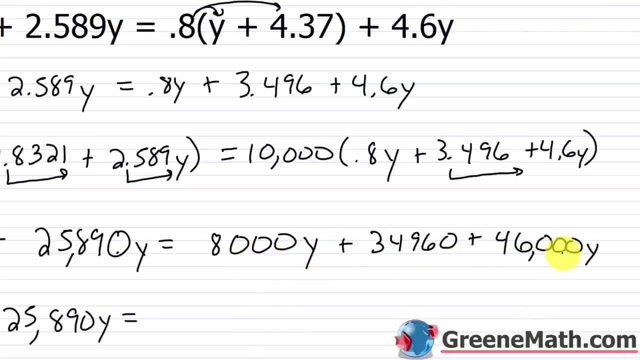 This is equal to, over here on the right, I can combine like terms. And I need to put a comma in there. I have 8,000y plus 46,000y. That's going to give me... 54,000y. 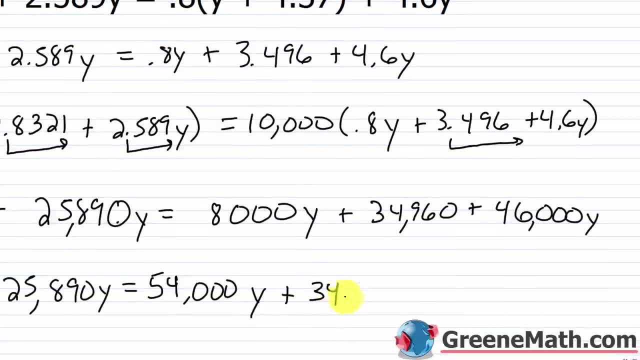 Then plus, and I put a comma in here, 34,960. 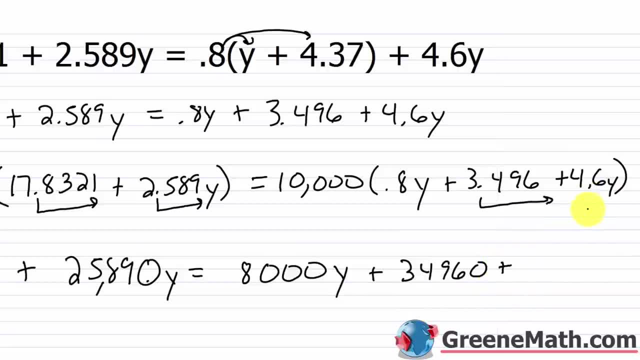 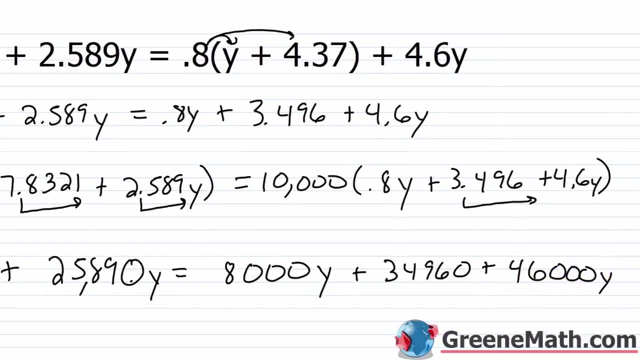 we have 4.6 y, so 10 000 times 4.6. we think about 46 here and i'm going to need to put three more zeros: one, two, three. this is going to go one, two, three, four places to the right, and then don't forget the y, and then we have 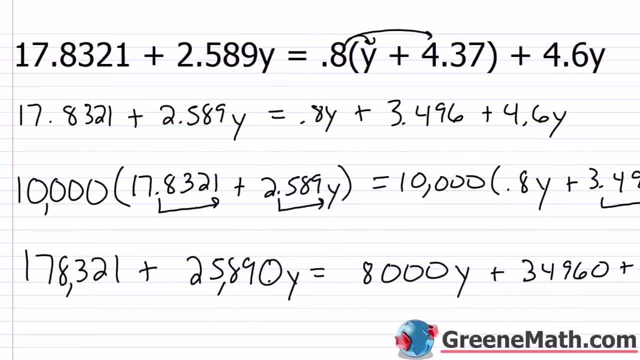 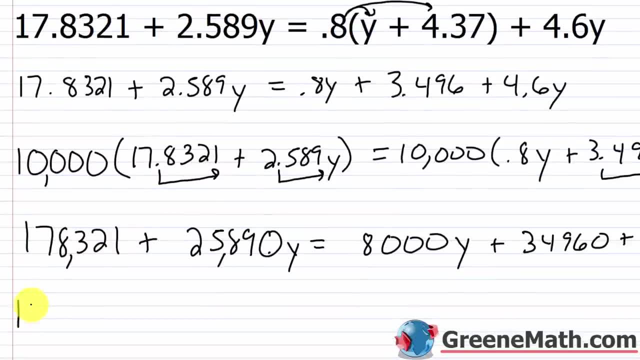 our transformed equation. unfortunately it's so big it doesn't fit on the screen. but we go through the same process on the left. i can't simplify any more, so i'm just going to write: 178 321 plus 25 890 y. this is equal to: 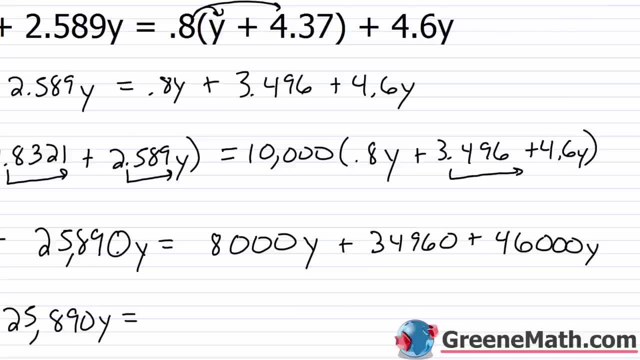 over here on the right. i can combine like terms and i need to put a comma in there. i have 8 000 y plus 46 000 y. that's going to give me 54 000 y, then plus- and i put a comma in here- 34 960. 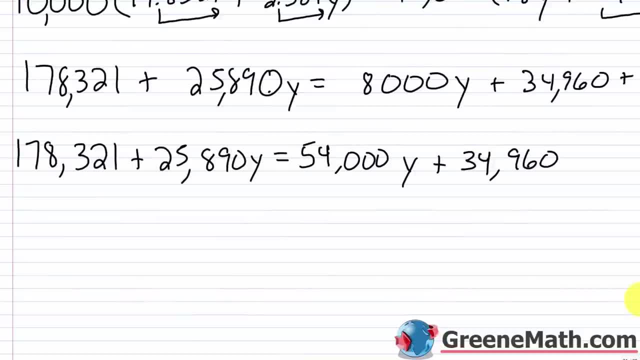 so again, i want all my variable terms on one side of the equation, and so i like my variable term to be on the left. i like my number to be on the right. so i'm going to go ahead and subtract 54 000 y from both sides of the equation. that's going to go away, and just to save a little time. 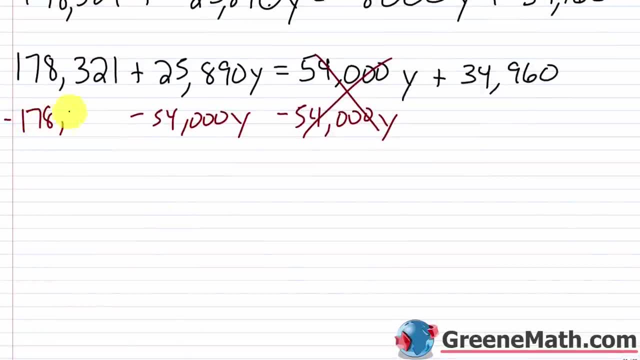 i'm going to simultaneously subtract 178- 321 from both sides of the equation. so why am i doing that? Well, what's going to end up happening is I'm going to have a variable term on this side, This is gone, and I'm just going to have a number on the right side. 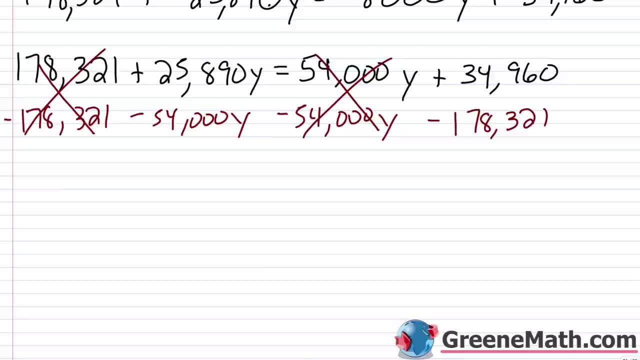 All right. so what is 25,890 minus 54,000? That's going to be negative 28,110,. and then y, And this is equal to what is 34,960 minus 178,321? That's going to give me negative 143,361. 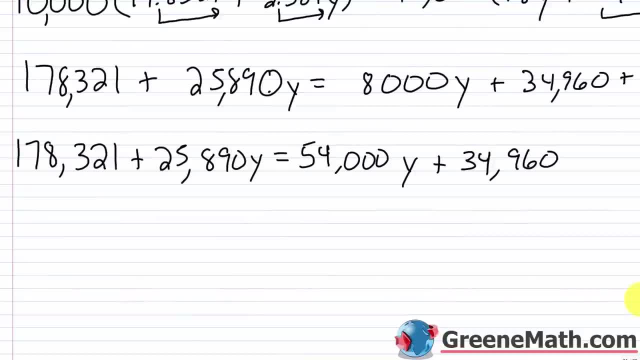 So again, I want all my variable terms on one side of the equation. And so I like my variable term to be on the left. I like my number to be on the right. 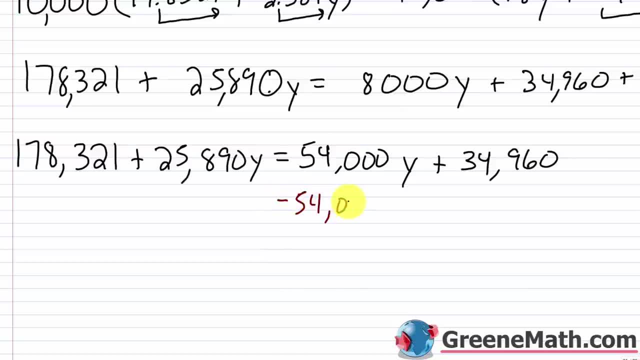 So I'm going to go ahead and subtract 54,000y from both sides of the equation. That's going to go away. 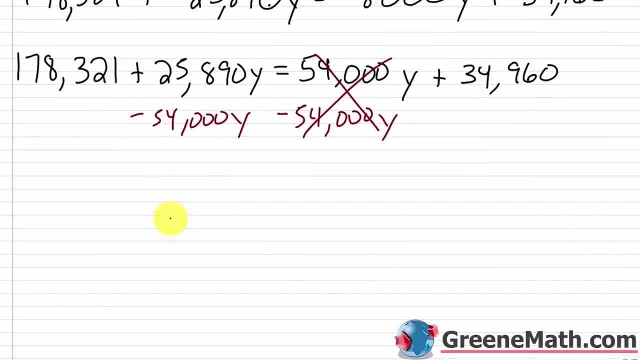 And just to save a little time, I'm going to simultaneously subtract 178,321 from both sides of the equation. 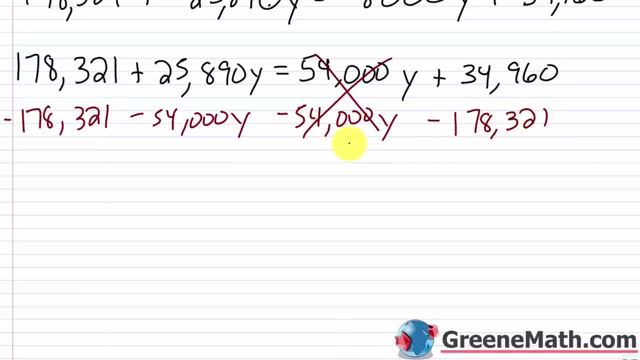 So why am I doing that? Well, what's going to end up happening is, I'm going to have a variable term on this side. This is gone. And I'm just going to have a number on the right side. 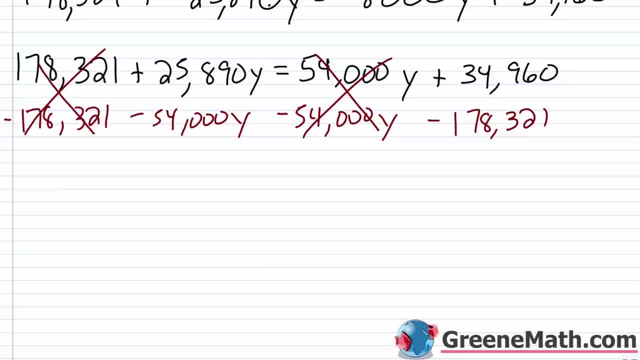 All right. So what is 25,890 minus 54,000? That's going to be negative 28,100. All right. So what is 25,890 minus 54,000? That's going to be negative 28,100. All right. So what is 25,890 minus 54,000? That's going to be negative 28,100. And then y. 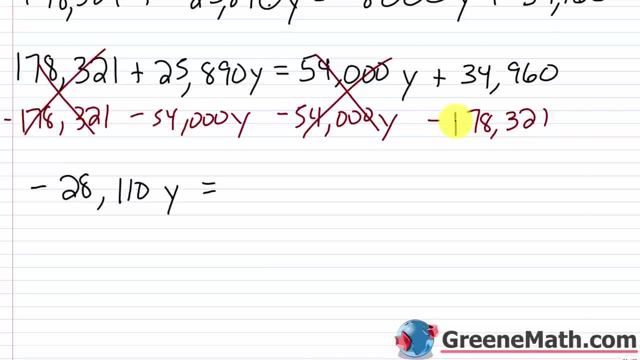 And this is equal to, what is 34,960 minus 178,321? 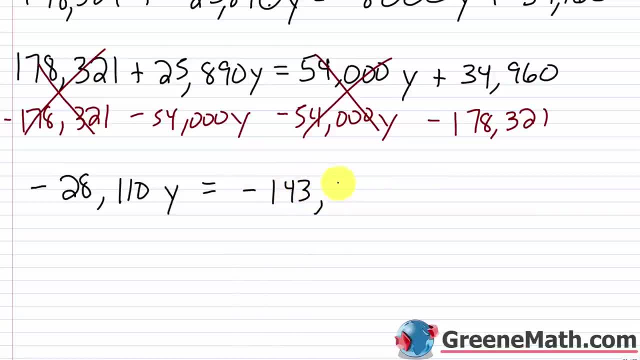 That's going to give me negative 143,361. 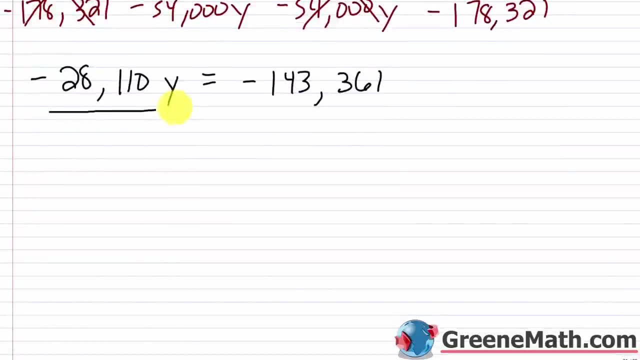 And now as a final step, we just get y by itself. We divide both sides of the equation by negative 28,110. Right? The coefficient of y. Negative 28,110. 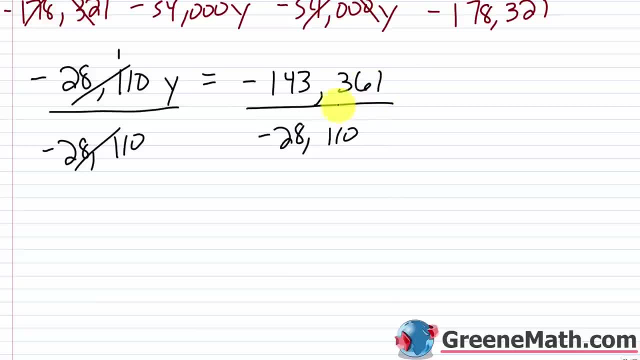 So negative 143,361. Divided by negative 28,110 is 5.1. So I'm going to have y equals 5.1. 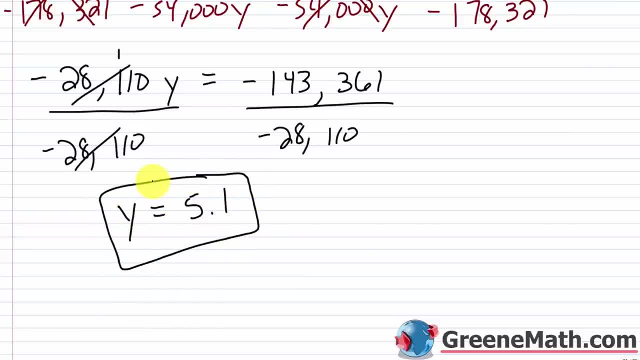 Now let's erase everything and we're going to check it. So again, y equals 5.1. 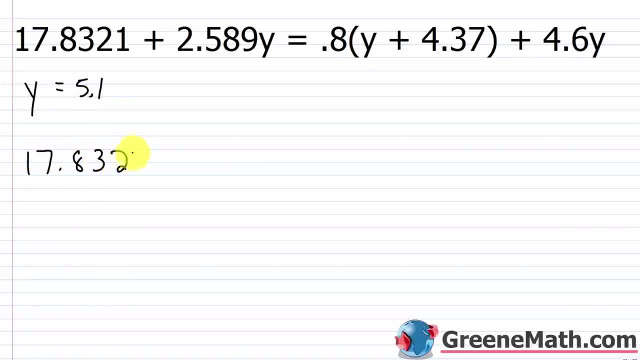 So I'm going to have 17.8321 plus 2.589 times 5.1 equals 0.8 times the quantity, for y I'm putting in 5.1, plus 4.37. Plus 4.6 times 5.1. 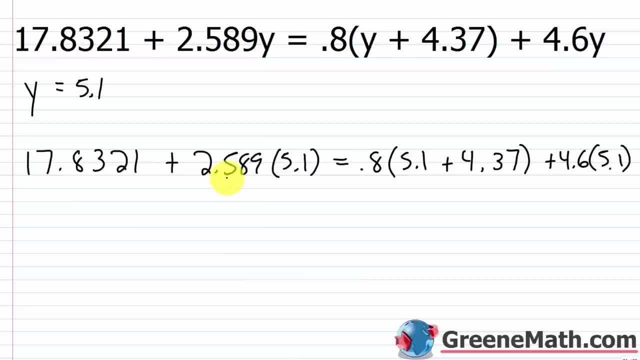 So starting on the left, 5.1 times 2.589 is 13.2039. 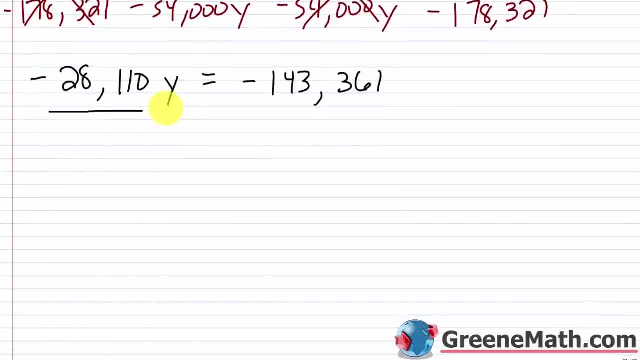 And now, as a final step, we just get y by itself. We divide both sides of the equation by negative 28,110, right the coefficient of y Negative 28,110.. So negative 143,361 divided by negative 28,110 is 5.1. 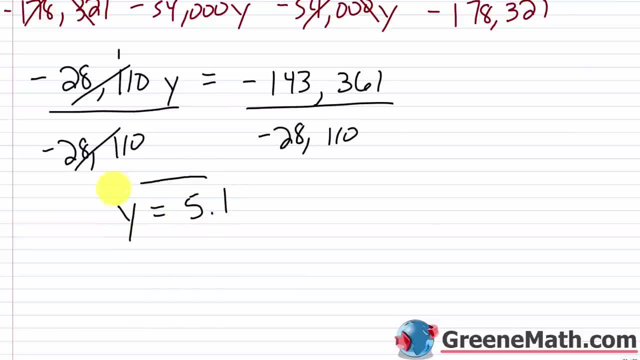 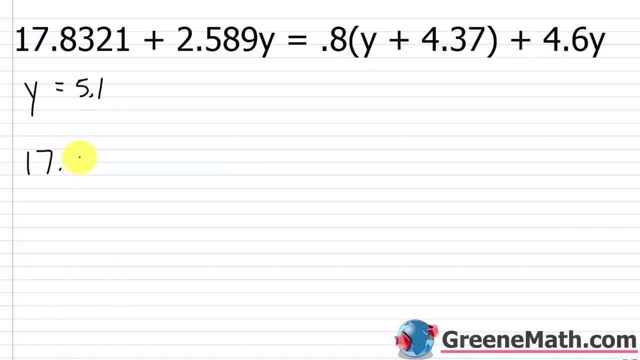 So I'm going to have y equals 5.1. Now let's erase everything and we're going to check it. So again, y equals 5.1.. So I'm going to have 17.8321 plus 2.589 times 5.1. 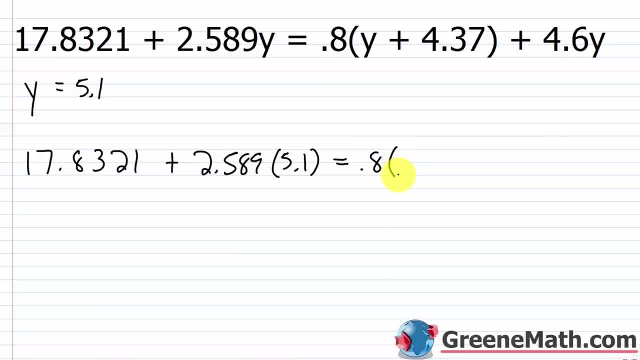 equals 0.8 times the quantity for y. I'm putting in 5.1 plus 4.37, plus 4.6 times 5.1. So, starting on the left, 5.1 times 2.589. Is 13.2039.. 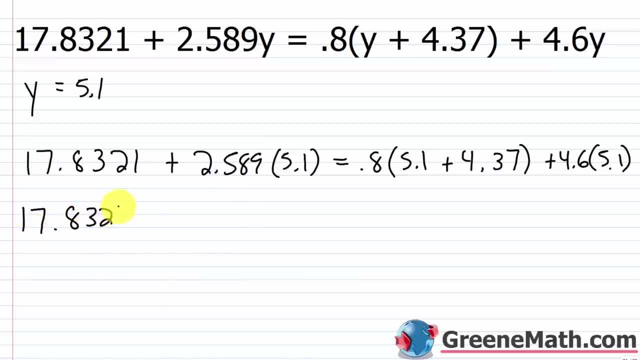 So I'd have 17.8321 plus 13.2039.. Now if I add these two, 17.8321 plus 13.2039 is going to give me 31.036.. Now over here I have 5.1 plus 4.37 to be done first. 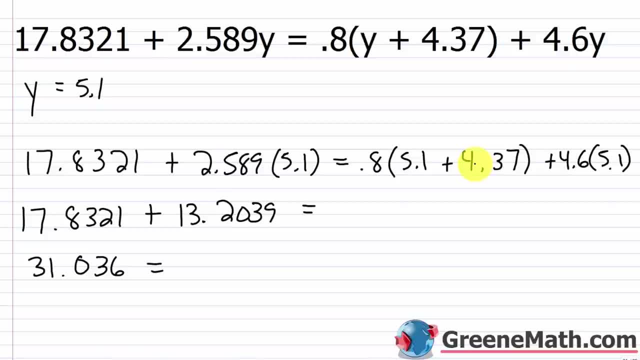 That's going to give me 9.47.. And if I multiply that by 0.8, I'm going to get 7.576.. Now, plus 4.6 times 5.1,, that gives me 23.46.. 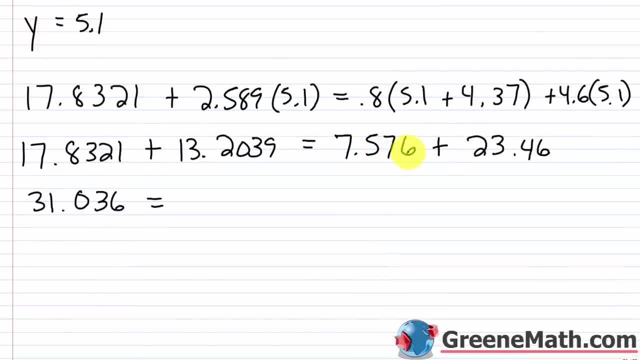 And if I combine these two, so 7.576 plus 23.46, I'm going to end up with 31.036.. So the same number on both sides of the equation. So I know my solution: y equals 5.1 is correct. 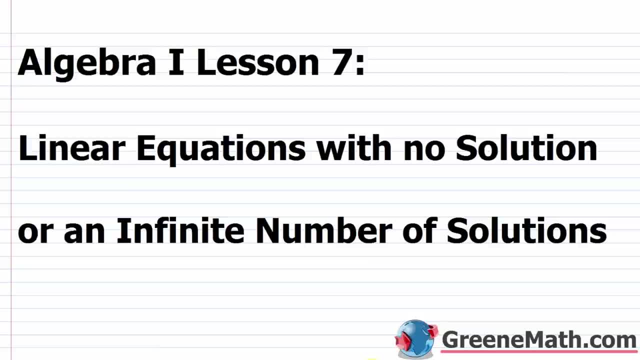 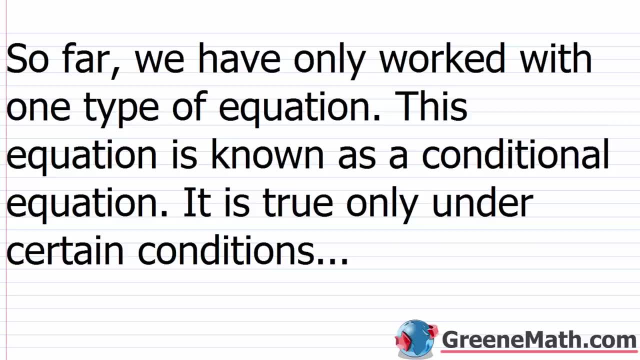 Hello and welcome to Algebra 1 Lessons. In this video we're going to learn about linear equations with no solution or an infinite number of solutions. All right, so so far we have only worked with one type of equation. This equation is known as a conditional equation. 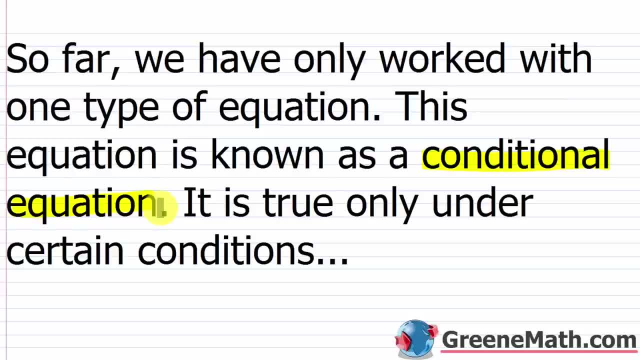 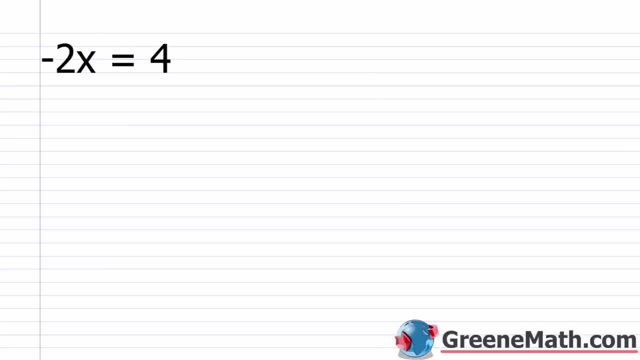 Let me highlight that a conditional equation, So it is true only under certain conditions. So let's see an example. So here's a very simple example of a conditional equation. Everything we've worked with so far has been a conditional equation. So negative 2x equals 4.. 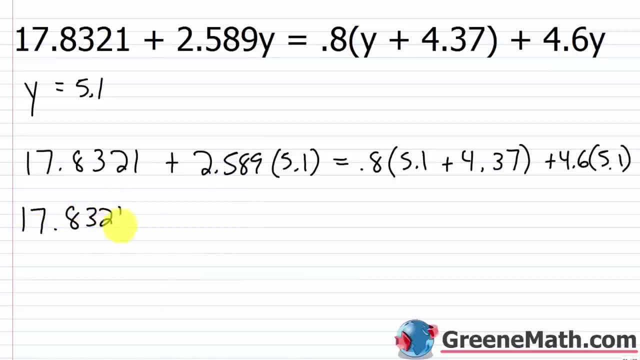 So I'd have 17.8321 plus 13.2039. 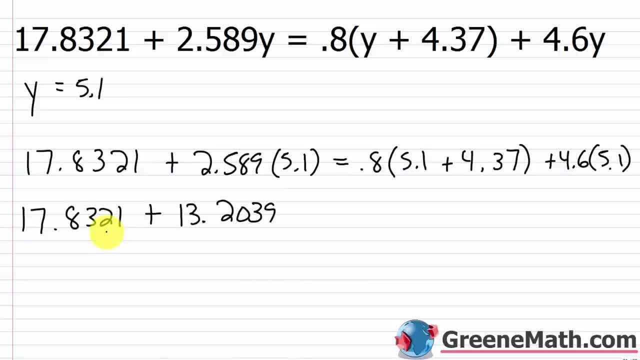 Now if I add these two, 17.8321 plus 13.2039 is going to give me 31.036. 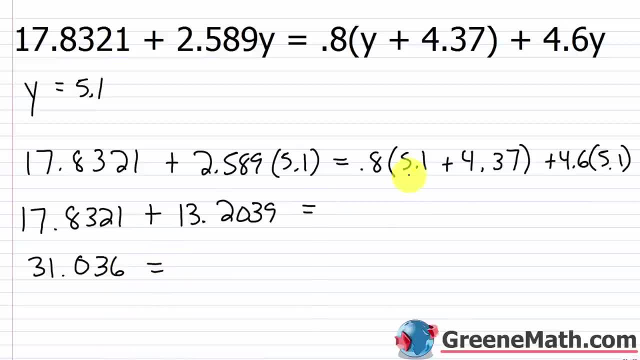 Now over here, I have 5.1 plus 4.37 to be done first. That's going to give me 9.47. 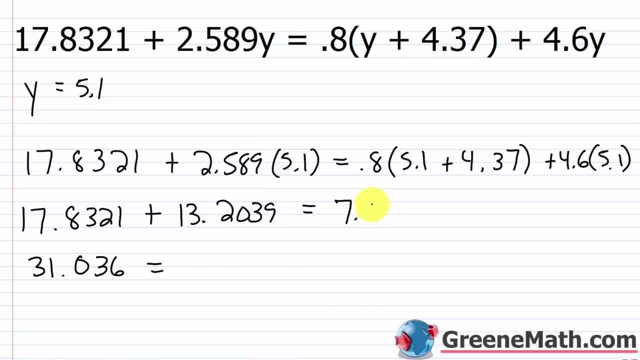 And if I multiply that by 0.8, I'm going to get 7.576. 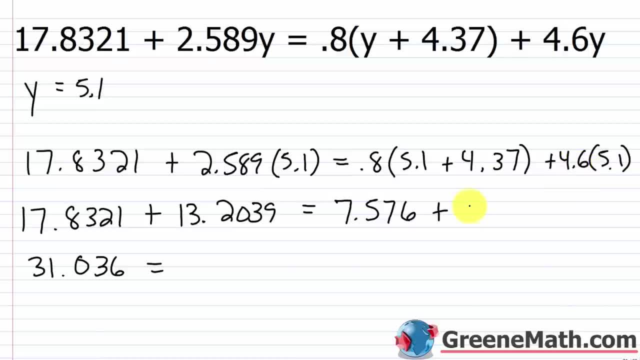 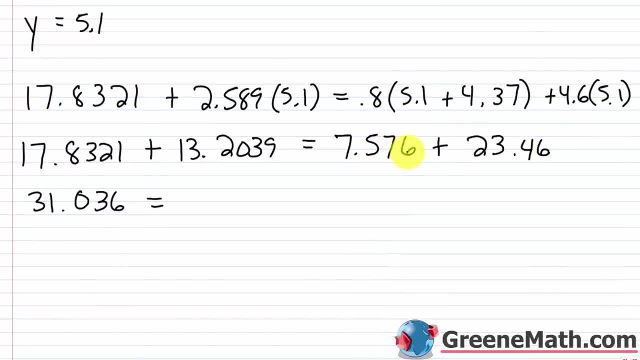 Now plus 4.6 times 5.1, that gives me 23.46. And if I combine these two, so 7.576 plus 23.46, I'm going to end up with 31.46. 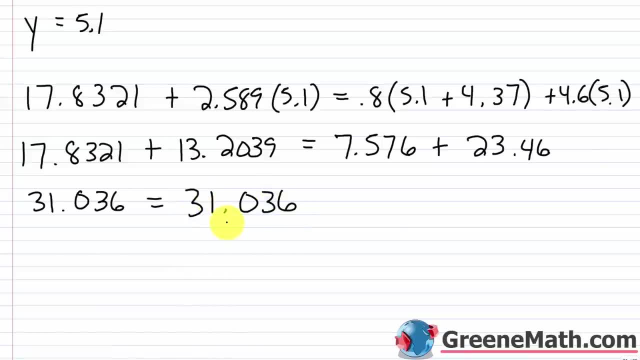 So the same number on both sides of the equation. Hello, and welcome to Algebra 1 Lesson 7. 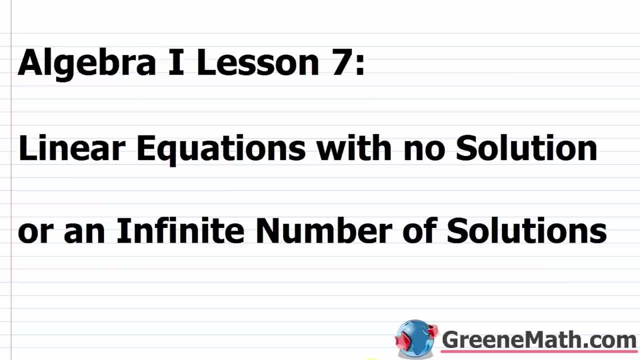 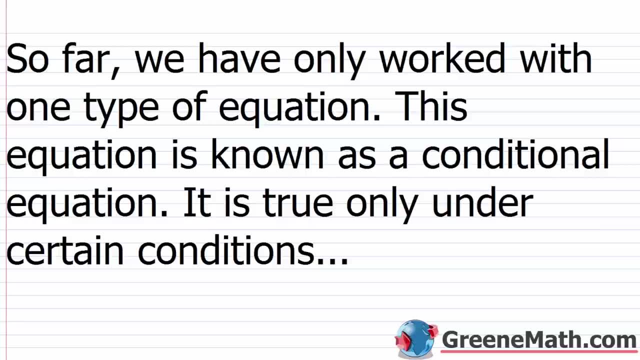 In this video, we're going to learn about linear equations with no solution, or an infinite number of solutions. All right, so so far, we have only worked with one type of equation. This equation is known as a conditional equation. Let me highlight that, a conditional equation. So it is true only under certain conditions. So let's see an example. 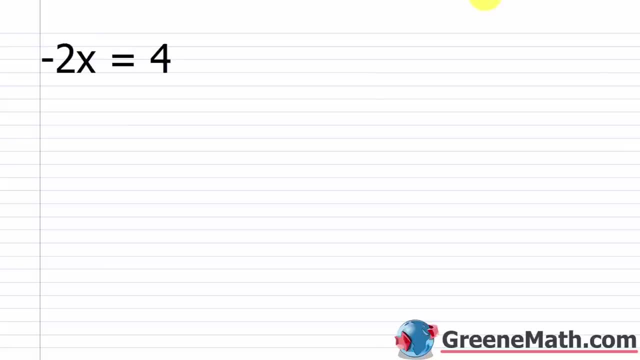 So here's a very simple example of a conditional equation. Everything we've worked with so far has been a conditional equation. So negative 2x equals 4. So we all know how to solve this at this point, right? We want to isolate x. So we divide both sides of the equation by negative 2, right? The coefficient of x. This cancels with this and becomes 1. So I have x equals 4 divided by negative 2 is negative 2. So that's my solution. 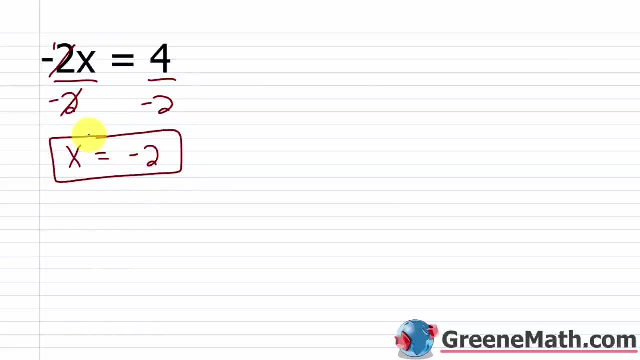 Now, the reason it's called a conditional equation is because this equation is true under this specific condition, that x is equal to negative 2. If I plug in a negative 2 for x, I would have negative 2 times negative 2 equals 4. And then this left side simplifies to 4. So 4 equals 4. So that all checks out. 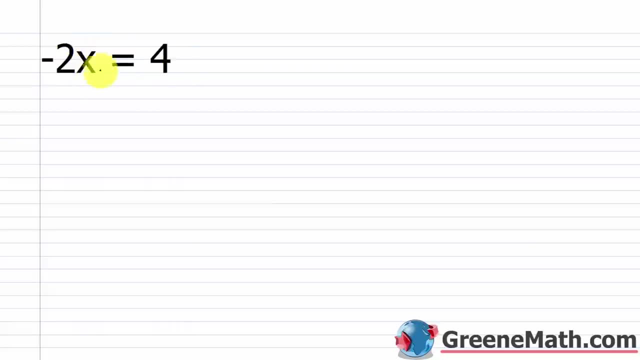 So we all know how to solve this at this point. right, We want to isolate x. So we divide both sides of the equation by negative 2, right, The coefficient of x. This cancels with this and becomes 1.. So I have: x equals 4 divided by negative. 2 is negative 2.. 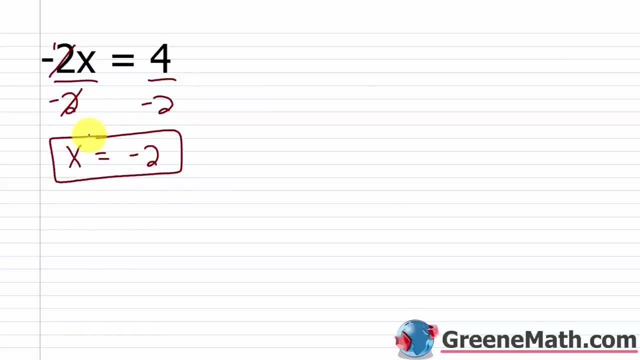 So that's my solution. Now, the reason it's called a conditional equation is because this equation is true under this specific condition that x is equal to negative 2.. If I plug in, If I plug in a negative 2 for x. 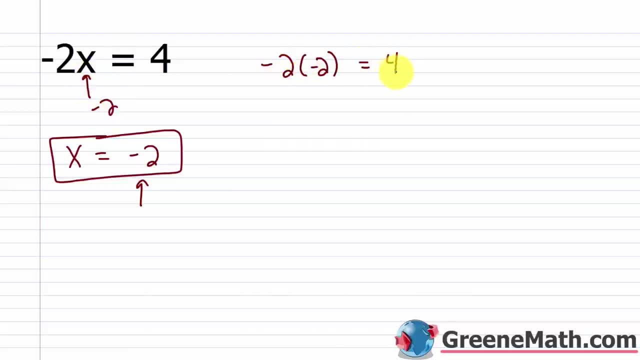 I would have negative 2 times negative. 2 equals 4.. And then this left side simplifies to 4.. So 4 equals 4.. So that all checks out. Now if I choose anything else for x. this is no longer a true statement. 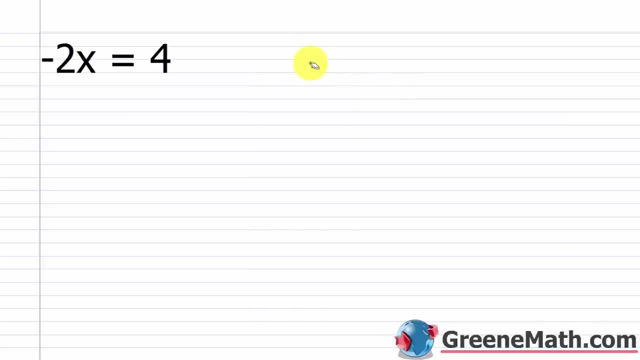 If I was to say, if I was to say, x is equal to 7,, for example? well, negative 2 times 7 is not equal to 4.. Negative 2 times 7 is not equal to 4.. Well, negative 2 times 7 is not equal to 4.. 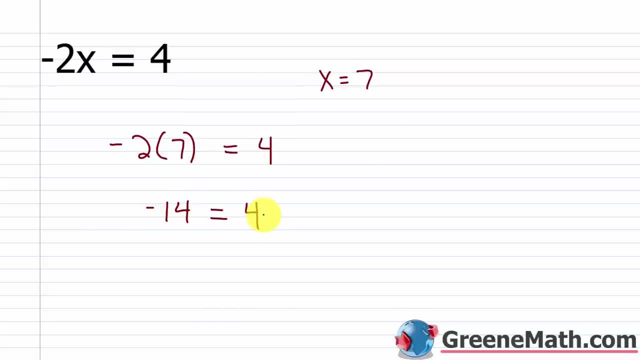 Well, negative 2 times 7 is negative 14.. That's not equal to 4.. This is wrong, wrong, okay. Only if I use x equals negative 2 will this equation be true. All right, so the next type of equation is known as an identity. 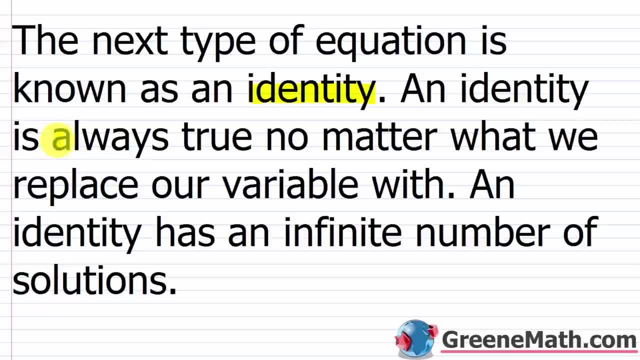 Okay, an identity. An identity is always true, okay, no matter what we replace our variable with. So we can replace it with a billion negative 2, 4, 27.. So we can replace it with a billion negative 2, 4, 27.. 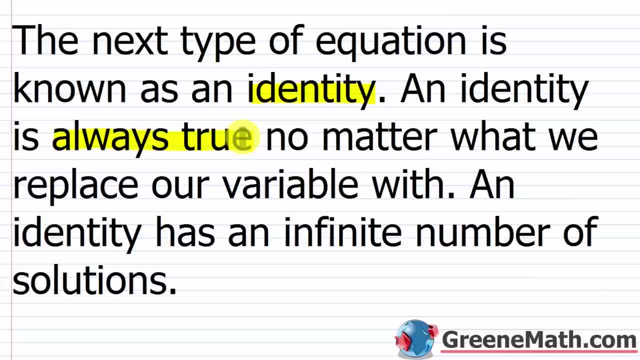 So we can replace it with a billion negative 2,, 4, 27.. Negative 1, 4th, it does not matter, it will always be true. The key thing is that an identity has an infinite number of solutions. 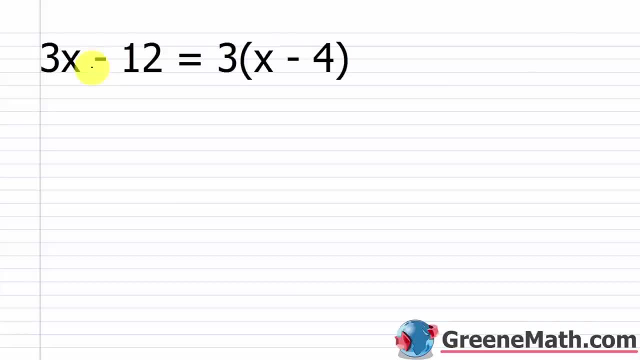 So here's an example of an identity. So we have 3x minus 12 equals 3 times the quantity x minus 4.. And before we go through and show why this is an identity, just in your head, pick any number you want. 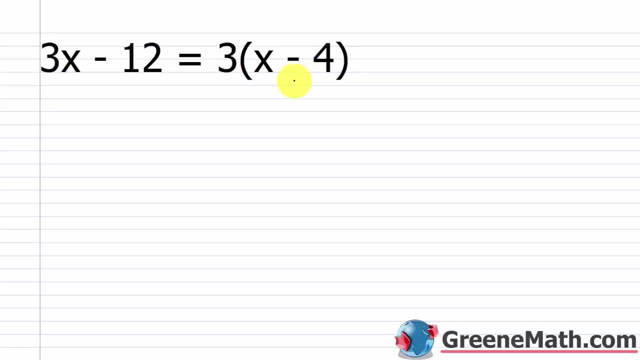 Doesn't matter what it is, and plug it in for x and I bet it works. I'm going to pick the number I don't know: negative 8.. So I'm going to plug in a negative 8 here and a negative 8 here. 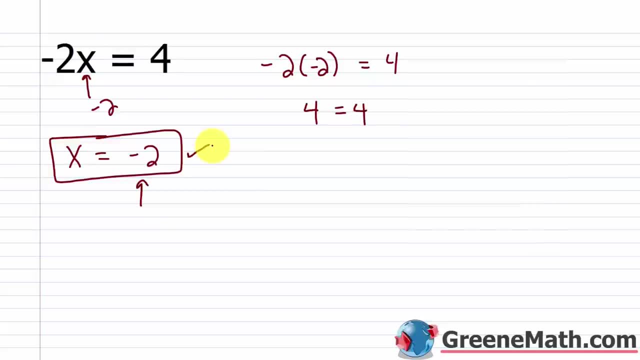 Now, if I choose anything else for x, this is no longer a true statement. If I was to say, 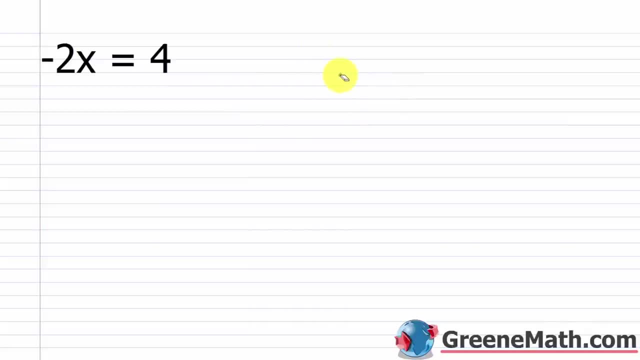 if I was to say, x is equal to 7, for example. 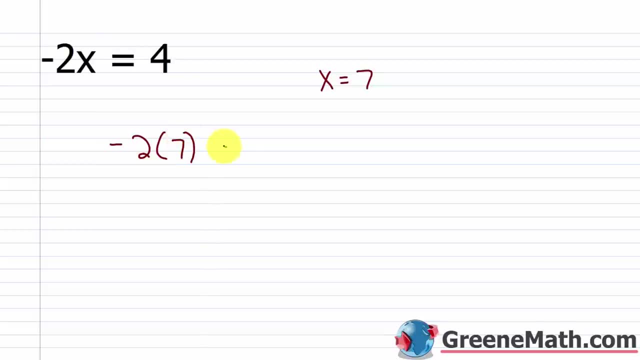 Well, negative 2 times 7 is not equal to 4. Negative 2 times 7 is negative 14. That's not equal to 4. This is wrong. Wrong. Okay? 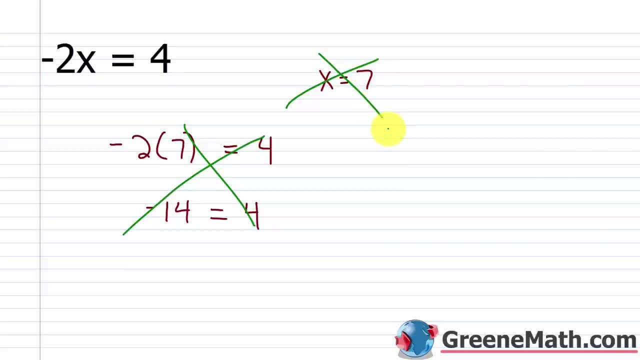 Only if I use x equals negative 2 will this equation be true. All right. 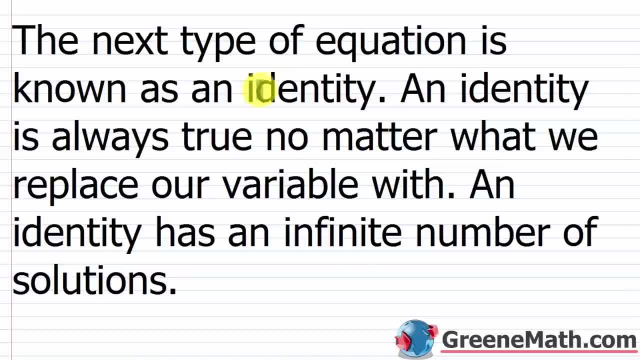 So the next type of equation is known as an identity. Okay? An identity is always true. Okay? No matter what we replace our variable with. 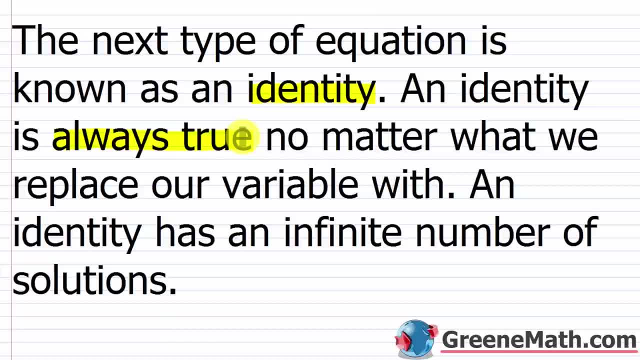 So we can replace it with a billion, negative 2, 4, 27, negative 1 fourth. It does not matter. 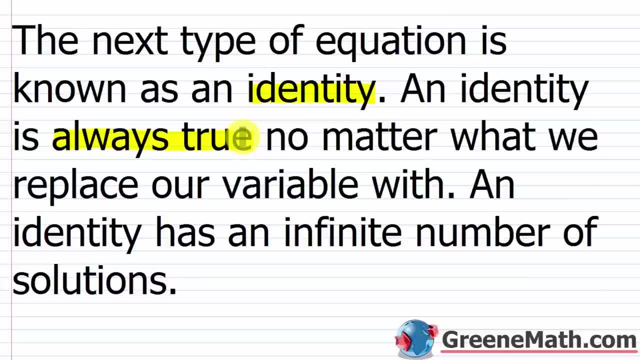 It will always be true. The key thing is that an identity has an infinite number of solutions. 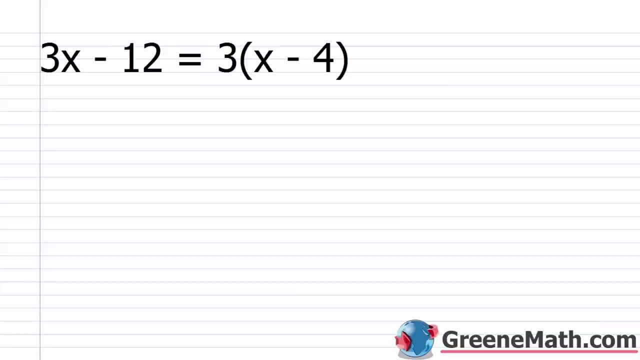 So here's an example of an identity. So we have 3x minus 12 equals 3 times the quantity x minus 12. equals 3 times the quantity x minus 4. And before we go through and show why this is an identity, just in your head pick any number you want. 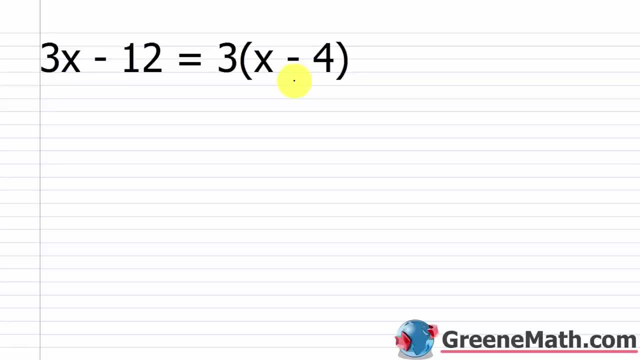 It doesn't matter what it is. And plug it in for x and I bet it works. 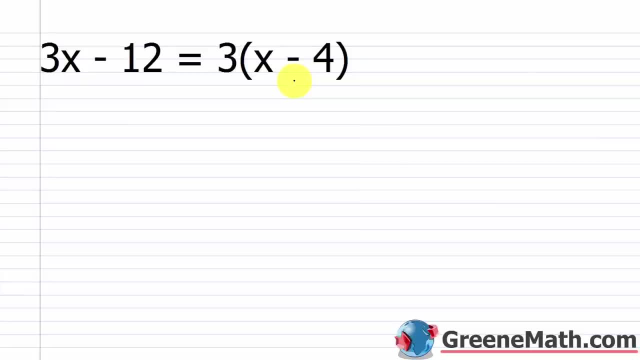 I'm going to pick the number, I don't know, negative 8. So I'm going to plug in a negative 8 here and a negative 8 here. And let's see if we get a true statement. 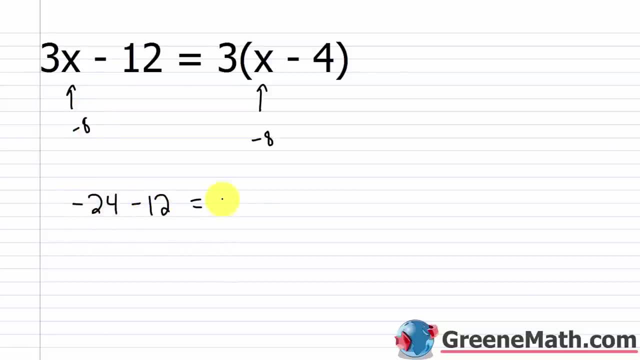 So 3 times negative 8 is negative 24 minus 12 equals 3 times the quantity negative 8 minus 4. So negative 8 minus 4. And negative 8 minus 4 is negative 12. So I would have 3 times negative 12 on the right. 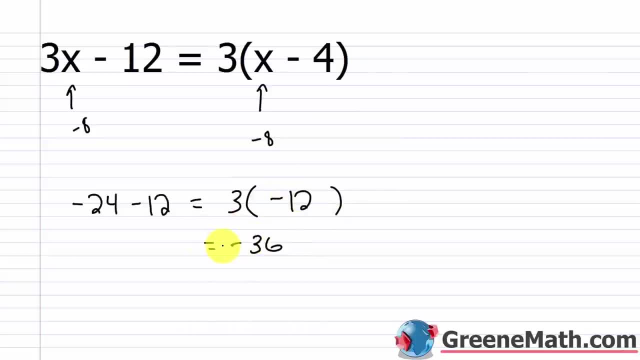 So this is negative 36. Over here, negative 24 minus 12 is negative 36 also. 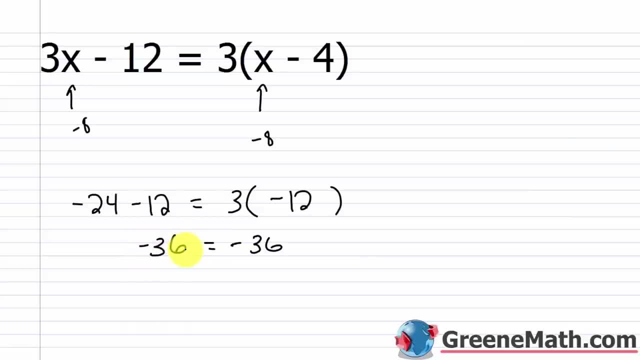 And you might say, okay, well you solved that already. You knew that x was equal to negative 8. 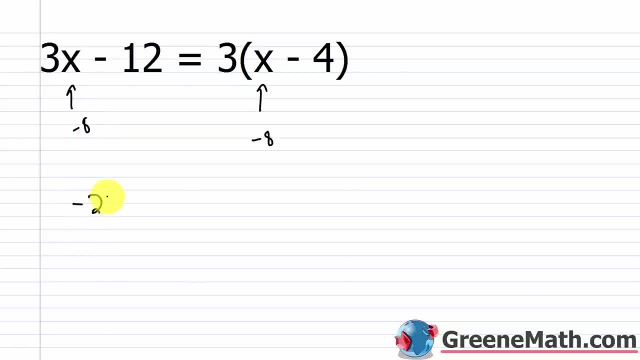 And let's see if we get a true statement. So 3 times negative 8 is negative. 24 minus 12 equals 3 times the quantity negative 8 minus 4.. So negative 8 minus 4.. And negative 8 minus 4 is negative 12.. 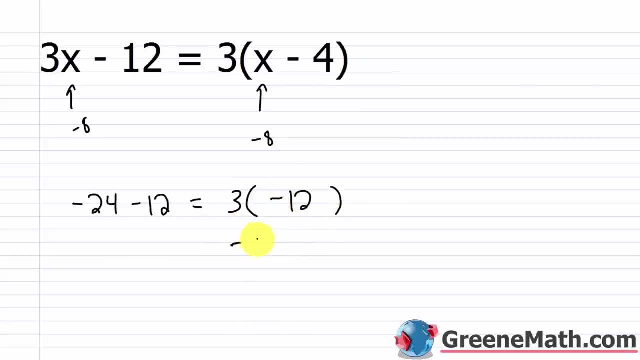 So I would have 3 times negative 12 on the right. So this is negative 36.. Over here, Negative 24 minus 12 is negative 36 also. And you might say: OK, well, you solved that already. You knew that x was equal to negative 8.. 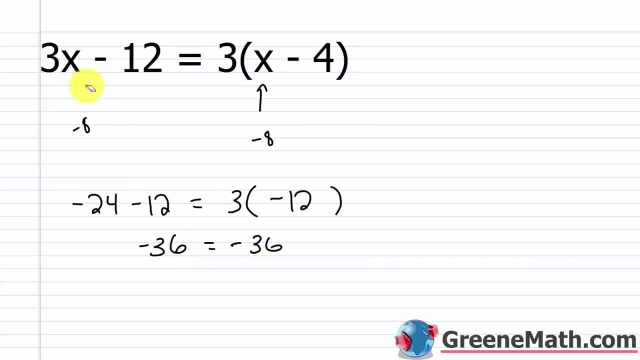 Pick anything else. Let's pick 4, for example. Let's pick 4 and see what happens. So I'll plug in a 4 here and I'll plug in a 4 here. So 3 times 4 is 12 over here minus 12.. 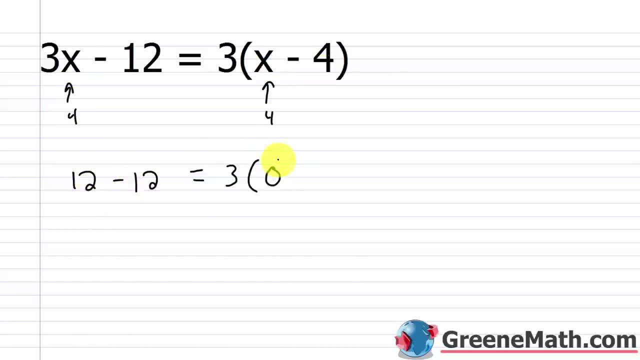 Over here I'll have 3 times the quantity 4 minus 4, which is 0.. So 3 times 0 is 0.. Over here, 12 minus 12 is 0.. 0 equals 0.. 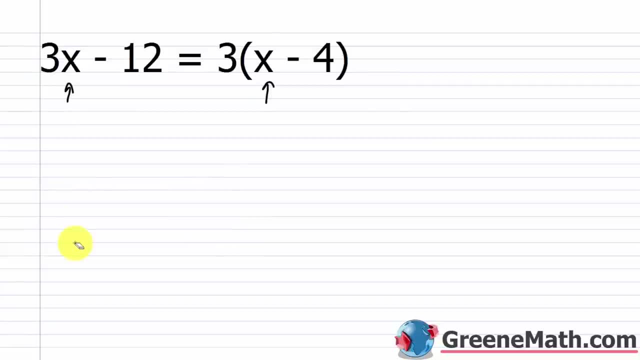 So that's a true statement. Let's try one more. So now let's try. I don't know. negative 3. Negative 3. So 3 times negative: 3 minus 12 is equal to 3 times the quantity negative 3 minus 4.. 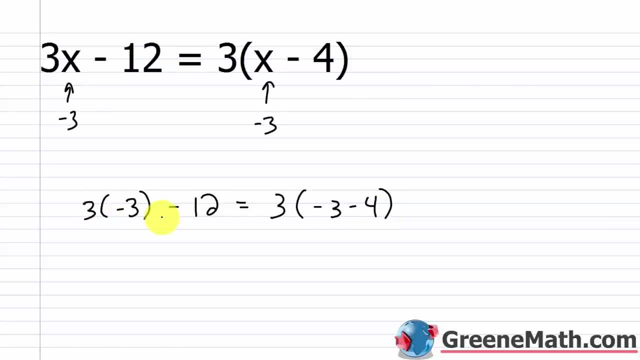 So over here: 3 times negative: 3 is negative 9.. Negative 9 minus 12 is negative 21.. Over here, 3 minus 4 is negative 7.. 3 times negative: 7 is negative 21.. So again, again, again. I get: the left and the right side is the same value. 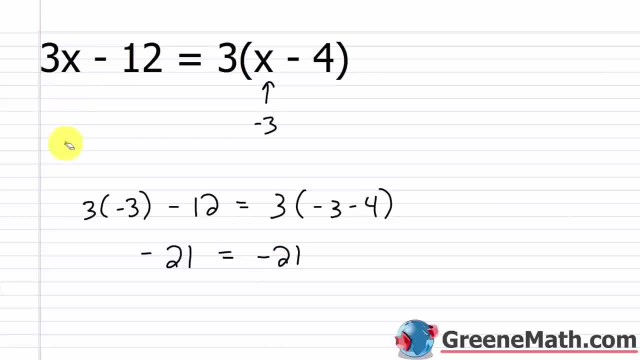 So how can that be the case? Well, the trick to this identity is, if you haven't noticed it already, the left and the right side are the exact same thing. They're just in different forms. This over here is just a simplified version of this over here. 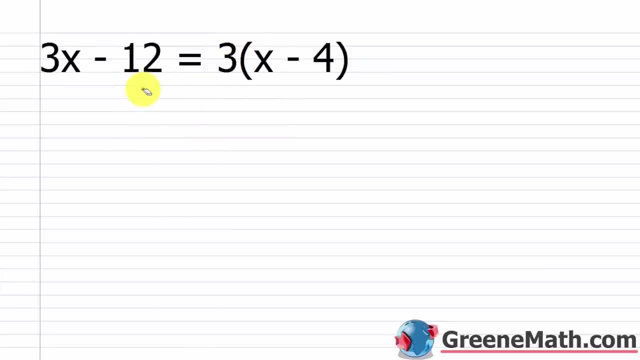 If I use my distributive property on the right side, so the left would still be 3x minus 12.. 3 times x is 3x, And then minus 3 times 4, that's 12.. So I have the exact same thing on both sides of the equation. 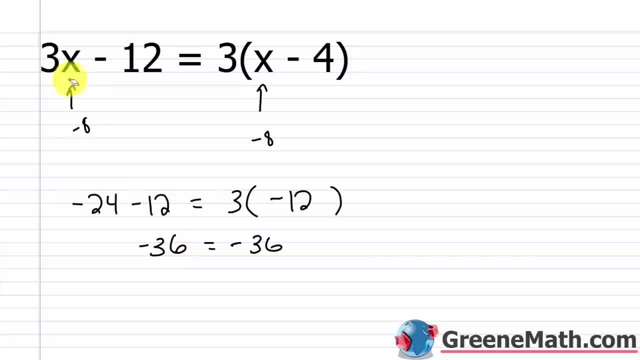 Pick anything else. Let's pick 4, for example. Let's pick 4 and see what happens. So I'll plug in a 4 here. And I'll plug in a 4 here. So 3 times 4 is 12 over here. Minus 12. 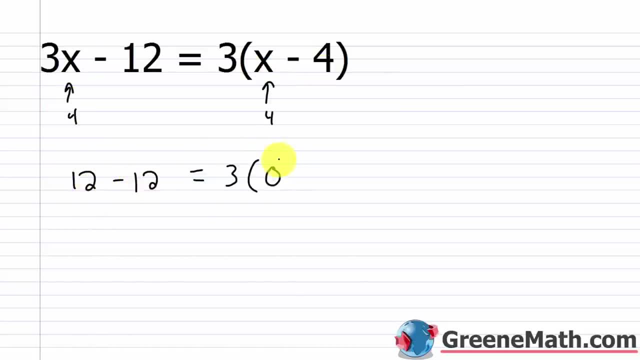 Over here, I'll have 3 times the quantity 4 minus 4, which is 0. So 3 times 0 is 0. Over here, 12 minus 12 is 0. 0 equals 0. So that's a true statement. Let's try one more. 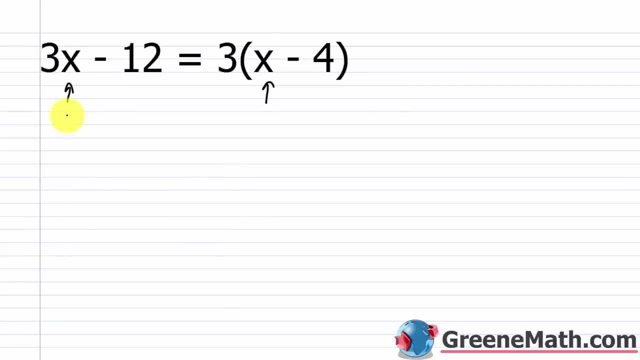 So now let's try, I don't know, negative 3. 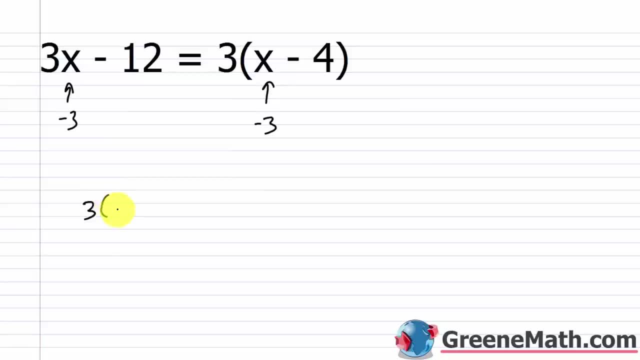 Negative 3. So 3 times negative 3 minus 12 is equal to 3. Times the quantity negative 3 minus 4. So over here, 3 times negative 3 is negative 9. Negative 9 minus 12 is negative 21. 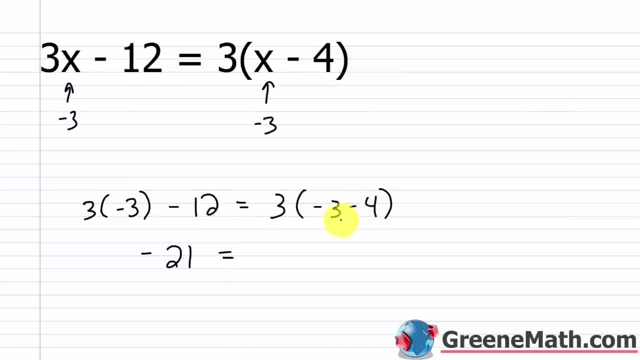 Over here, negative 3 minus 4 is negative 7. 3 times negative 7 is negative 21. 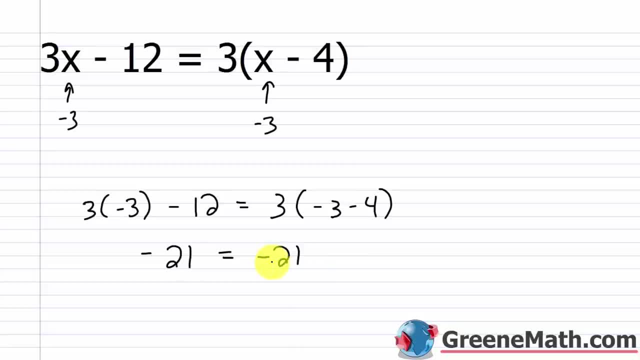 So again, again, again, I get the left and the right side is the same value. So how can that be the case? 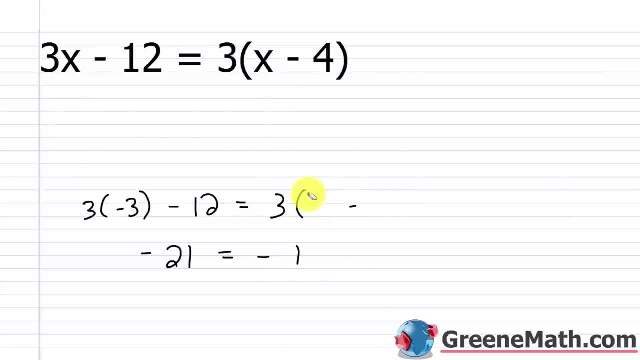 Well, the trick to this identity is, if you haven't noticed it already, the left and the right side are the exact same thing. 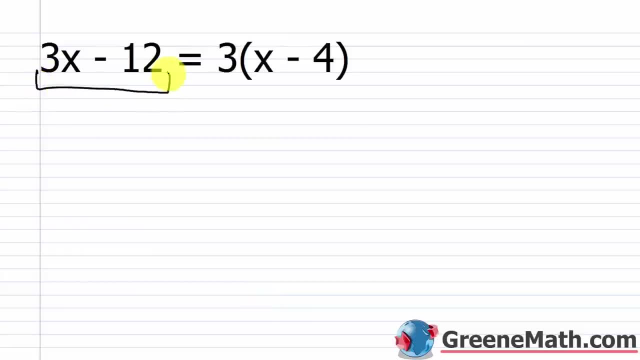 They're just in different forms. This over here is just a simplified version of this over here. 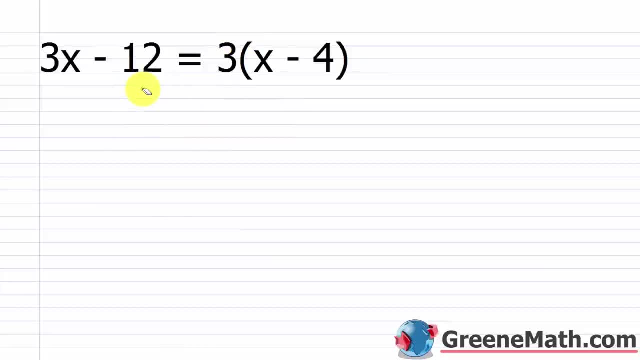 If I use my distributive property on the right side, so the left would still be 3x minus 12. 3 times x is 3x. And then minus 3 times 4, that's 12. So I have the exact same thing on both sides of the equation. So of course, whatever I plug in here and here, I'm going to get the same value because I'm doing the exact same thing. 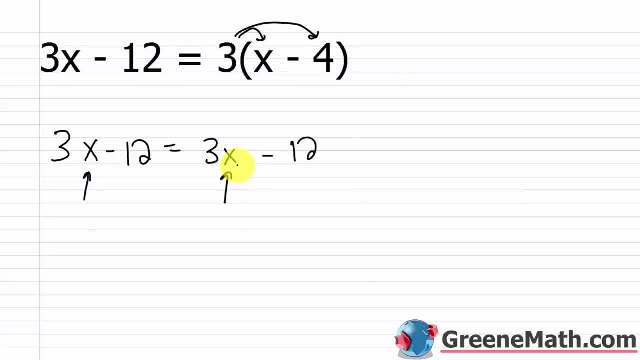 If I plug in a 2 here, and I plug in a 2 here, in each case, I'm multiplying 3 by 2, and then I'm subtracting away 12 on both sides. So it doesn't matter what number I pick. I do the exact same thing to it. And so the left and the right side will always be equal. And so there's an infinite number of solutions because I can choose any number that I want. 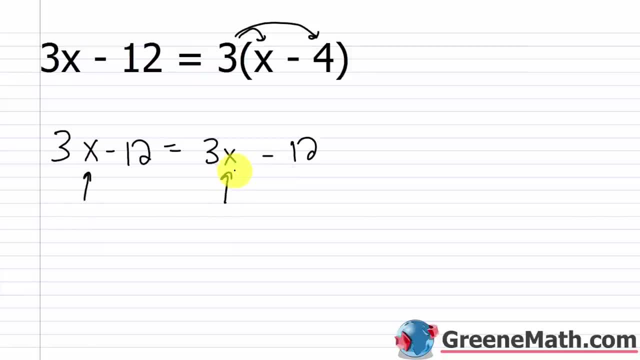 So, of course, whatever I plug in here and here, I'm going to get the same value right, Because I'm doing the exact same thing. If I plug in a 2 here and I plug in a 2 here, in each case, I'm multiplying 3 by 2 and then 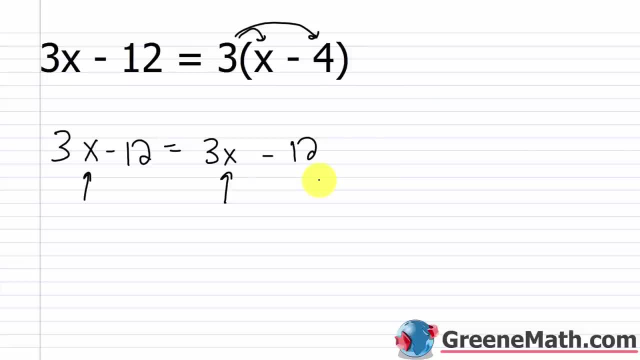 I'm subtracting away 12 on both sides, So it doesn't matter what number I pick, I do the exact same thing to it. Okay, The left and the right side will always be equal, And so there's an infinite number of solutions, because I can choose any number that I want. 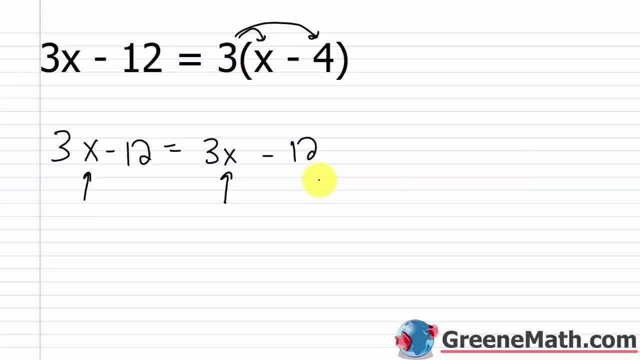 right. It's literally unlimited as far as how many solutions you would have. So if you were to come across this in your textbook or your teacher gives it to you for homework or a test, just write that the solution is all real numbers And as we move throughout algebra we're going to see some different notation that we're 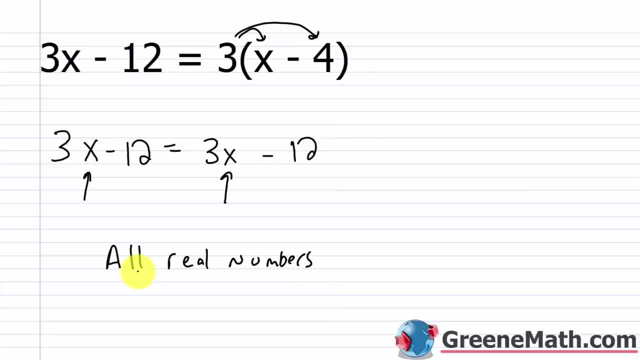 going to use to say: hey, all real numbers. Right, We're just going to write it out. Okay, We're not ready for the notation yet, So we're just going to write all real numbers. That's your solution, All right. 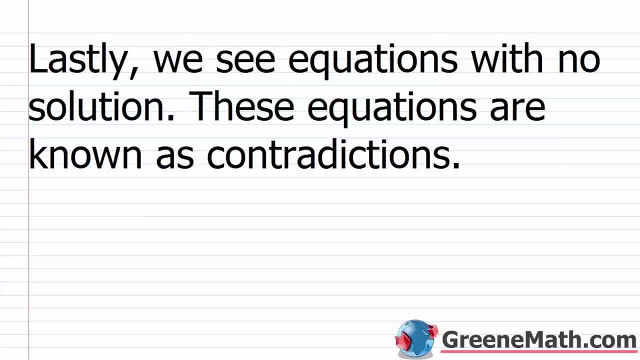 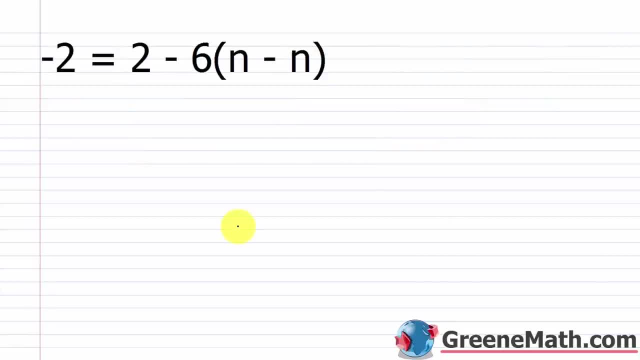 So, lastly, we see equations with no solution. These equations are known as contradictions, So contradictions. So no matter what you choose for n, it's never going to work. And to see why, let's simplify the right-hand side of the equation. 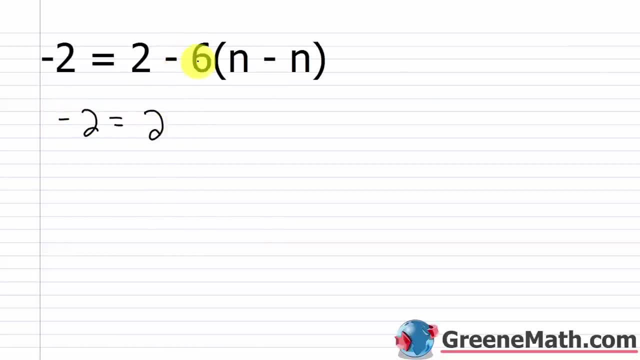 So negative 2 equals we have 2, we have negative 6 times n, That's negative 6n. Then we have negative 6 times negative n, That's positive 6n. So what you're going to see is that, if I simplify the right-hand side here, the variable n is: 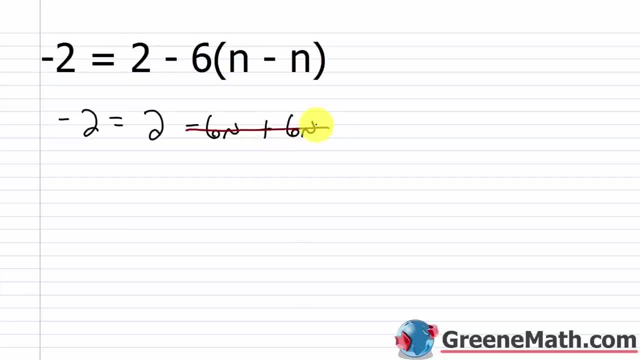 going to go away completely. Negative 6n plus 6n- those are opposites. Those are gone. So what I'm left with is just nonsensical statement that negative 2 equals 2. Well, it doesn't. This is wrong. 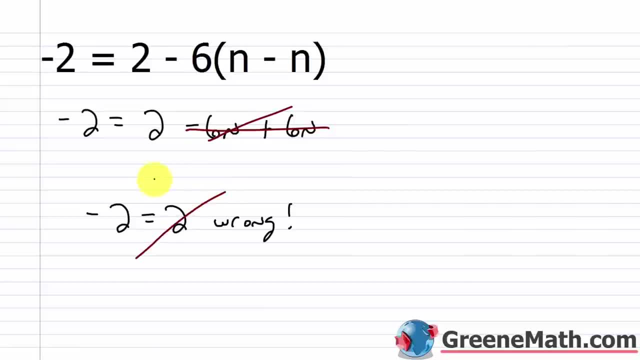 Negative 2 doesn't equal 2.. So nothing is ever going to work here. Right, This is what you do, Because if I put something in for n, I'm just going to subtract it away. So the result of this would be 0, right? 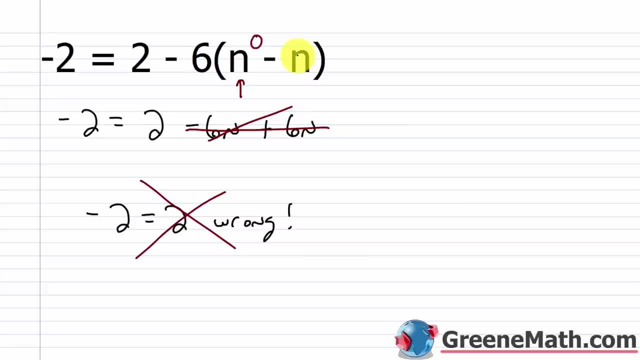 I plug something in for n. I subtract that same number away, I get 0.. I multiply 6 times 0, I get 0.. So I'm just left with negative. 2 equals 2, right once I simplify. 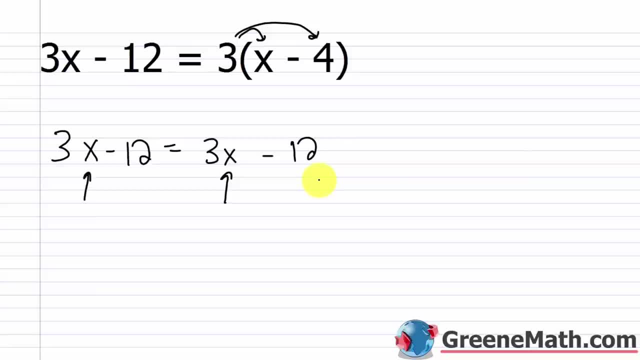 It's literally unlimited as far as how many solutions you would have. So if you were to come across this in your textbook 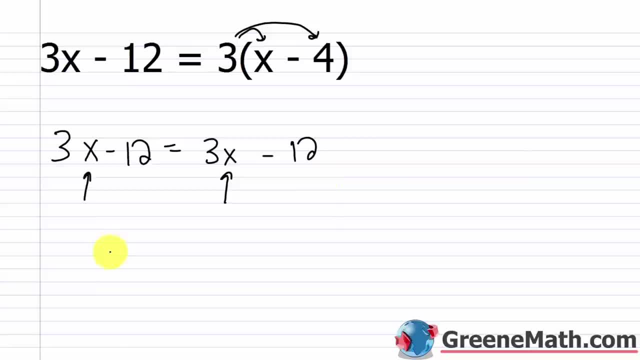 or your teacher gives it to you for homework or a test, just write that the solution is all real numbers. 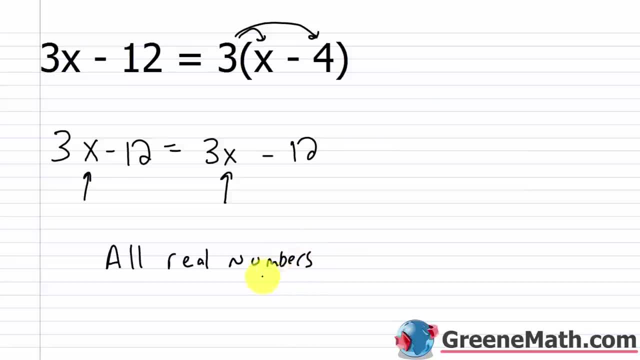 And as we move throughout algebra, we're going to see some different notation that we're going to use to say, hey, all real numbers. But right now, we're just going to write it out. We're not ready for the notation yet. So we're just going to write all real numbers. That's your solution. 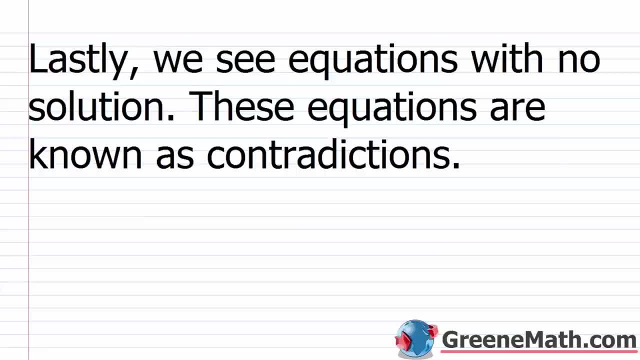 So lastly, we see equations with no solution. These equations are known as contradictions. 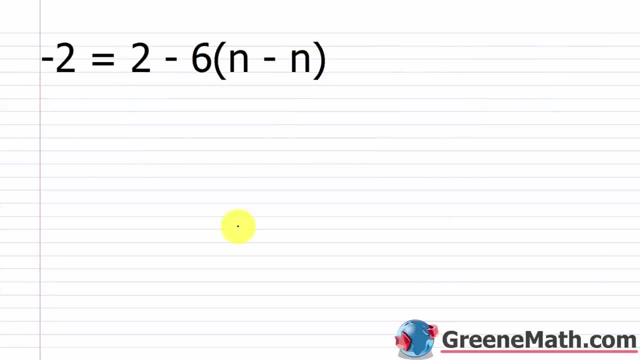 So contradictions. So no matter what you choose for n, 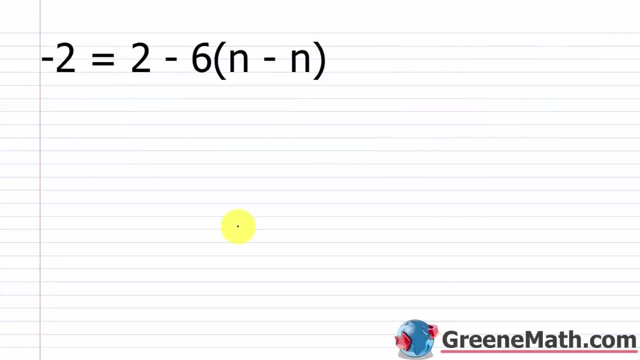 it's never going to work. And to see why, let's simplify the right-hand side of the equation. 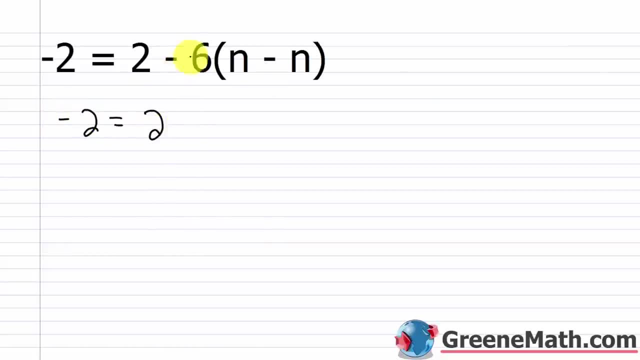 So negative 2 equals, we have 2, we have negative 6 times n. That's negative 6n. 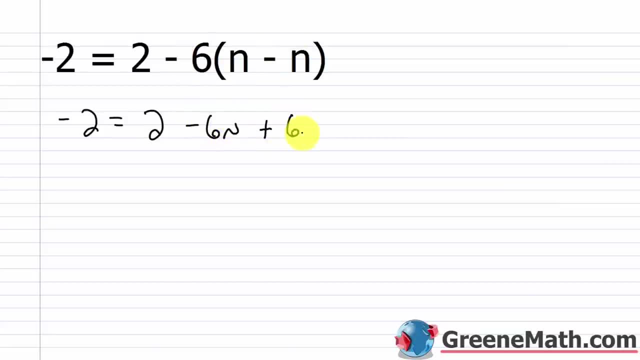 Then we have negative 6 times negative n. That's positive 6n. 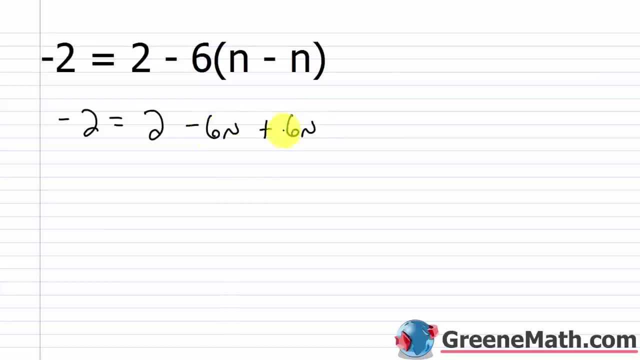 So what you're going to see is that if I simplify the right-hand side here, the variable n is going to go away completely. Negative 6n plus 6n, those are opposites. 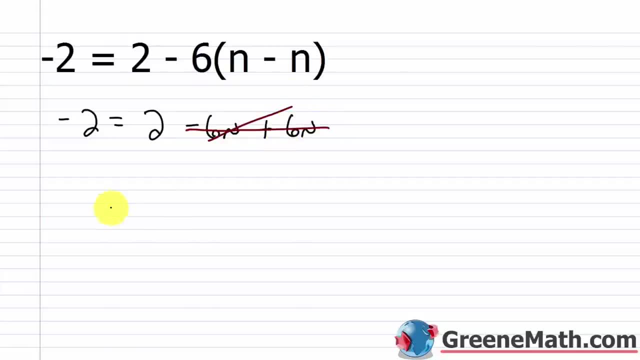 Those are gone. So what I'm left with is just nonsensical statement 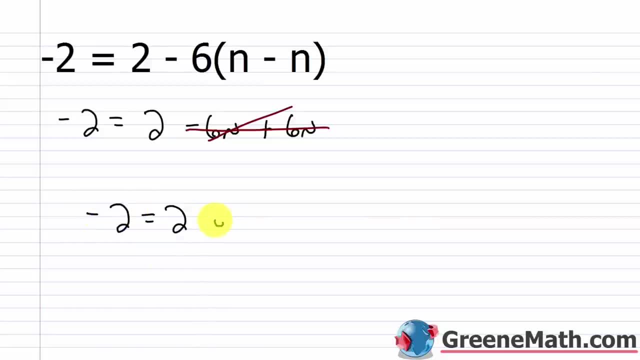 that negative 2 equals 2. Well, it doesn't. This is wrong. 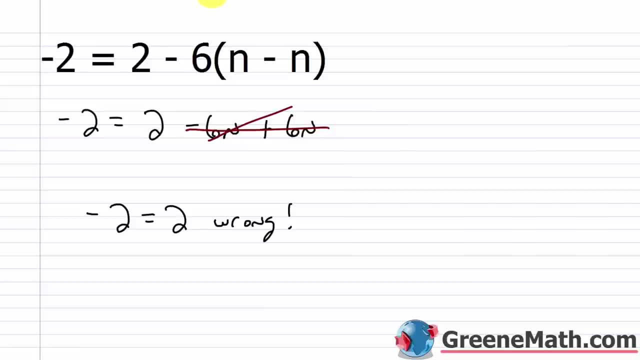 Negative 2 doesn't equal 2. So nothing is ever going to work here, right? 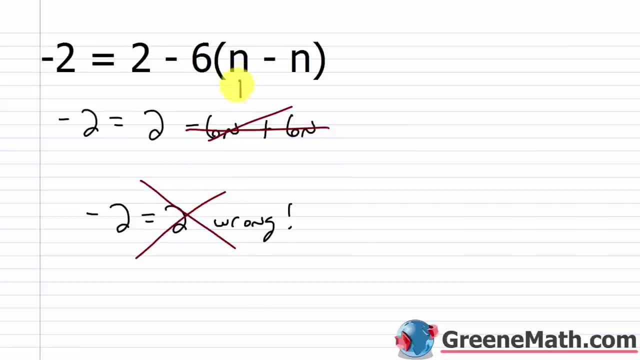 No matter what you do. Because if I put something in for n, I'm just going to subtract it away. 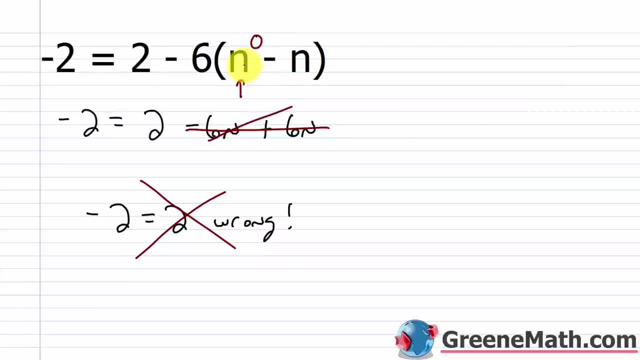 So the result of this would be 0, right? I plug something in for n. I subtract that same number away. I get 0. 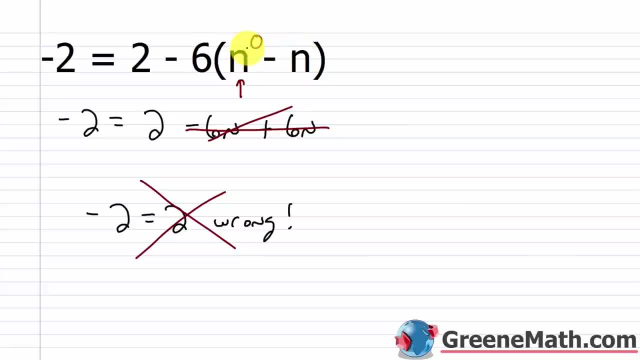 I multiply 6 times 0. I get 0. So I'm just left with negative 2 equals 2, right? Once I simplify. This is what I'm going to have. 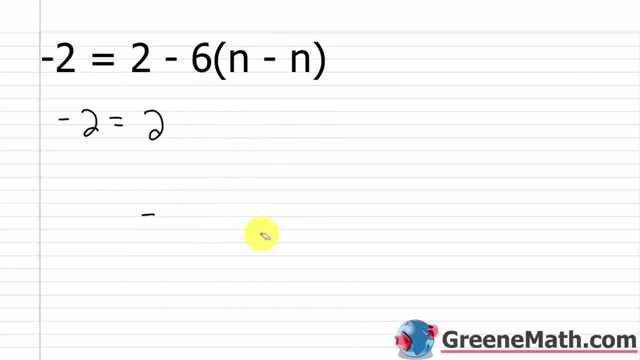 This is what I'm going to have, no matter what I choose for n. Negative 2 equals 2.. So there's no value of n that can ever be chosen. That will make this a true statement, And so this is an example of a contradiction. 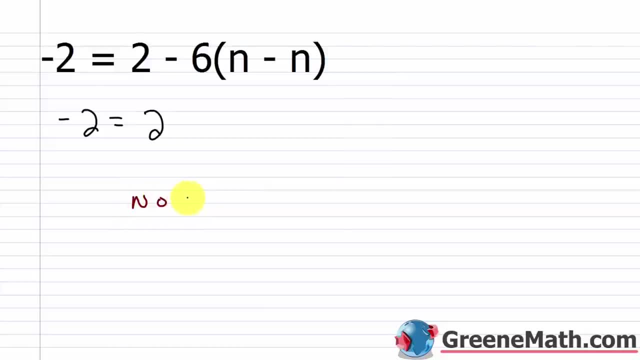 And so when this occurs, you can put no solution, And again we'll have some fancy notation for that moving forward, But for right now just put no solution. Hey, there's nothing I can do here. So let's look at some examples and let's see if we can figure out through simplification. 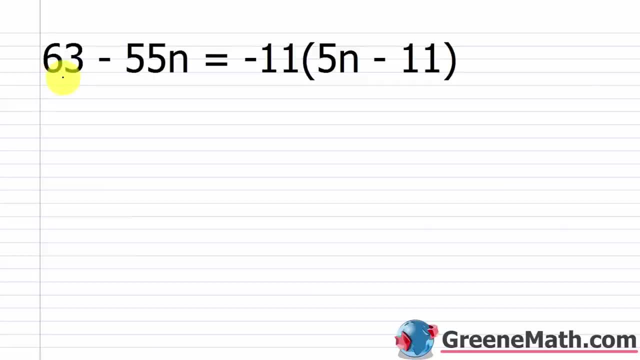 what type of equation they are. So this one I have 63 minus 55n equals negative 11. And I'm going to put that here. I'm going to put that here, I'm going to put that here: Negative 11 times this quantity: 5n minus 11.. 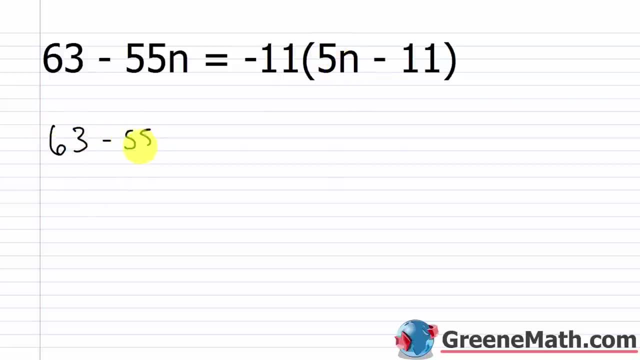 So on the left, 63 minus 55n. On the right, I'm going to use my distributive property to remove the parentheses. So negative 11 times 5n, That's negative 55n, And then I'll have negative 11 times negative 11.. 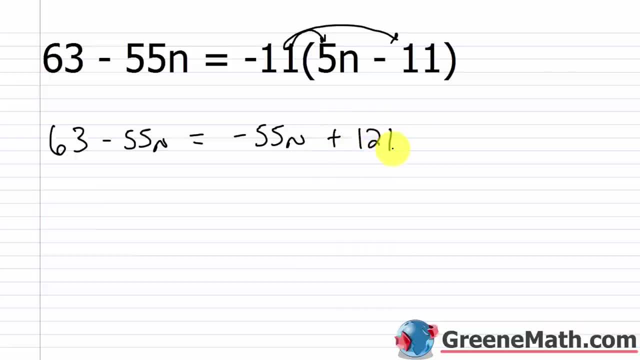 That's positive 121.. I told you this in one of the videos I made in a previous lesson or practice that I can't remember which one. if you have the exact same number on two sides of the equation, you can get rid of it In other. 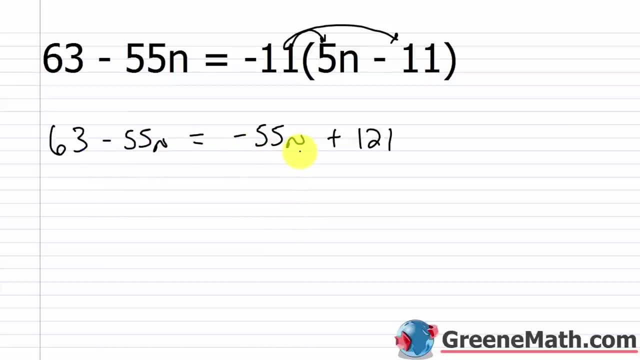 words, I have negative 55N here. I have negative 55N here. I can just get rid of it. Why is that the case? Well, through the addition property of equality, I can legally make it disappear. If I add 55N here and I add 55N here, I've added the same number to both sides of the equation. 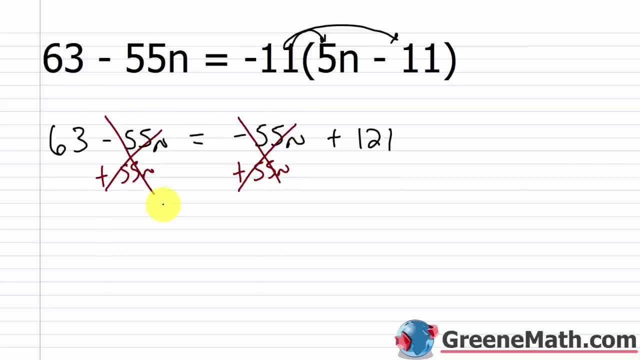 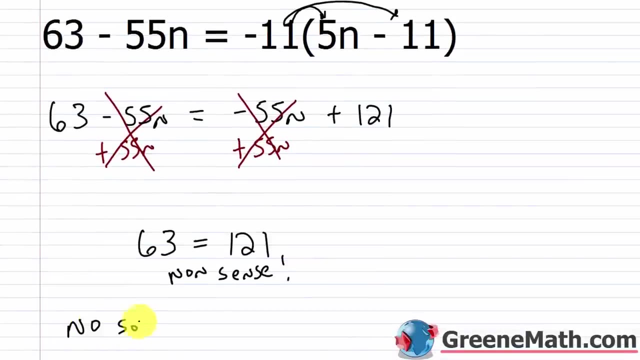 In both cases it's gone. It sums to zero and I'm left with 63 equals 121, which again is nonsense. This is nonsense, Okay, In case you don't know. So there's no solution here. No solution, This. 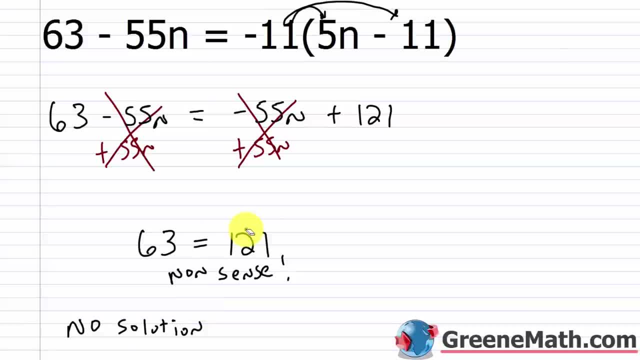 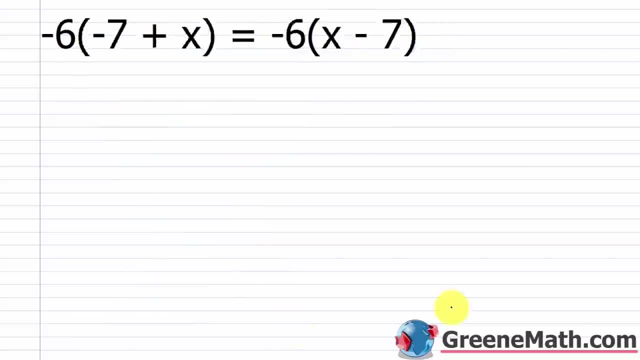 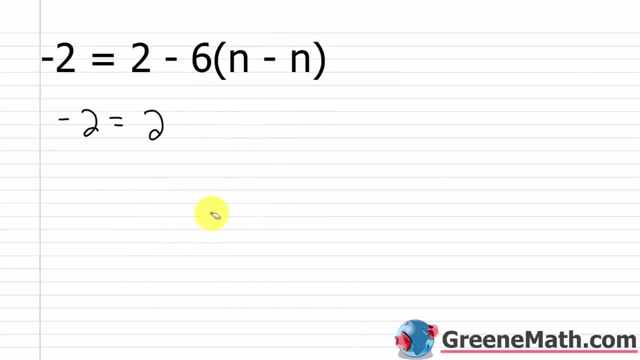 No matter what I choose for n. Negative 2 equals 2. So there's no value of n that can ever be chosen that will make this a true statement. 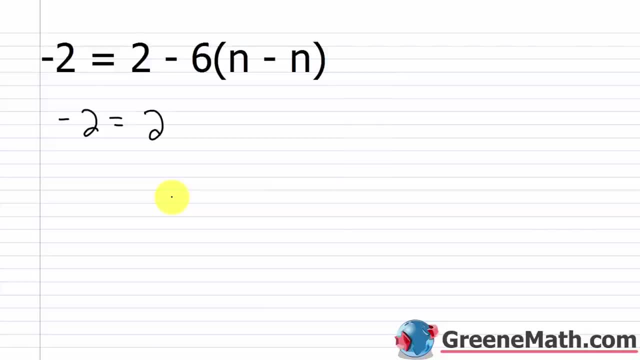 And so this is an example of a contradiction. And so when this occurs, 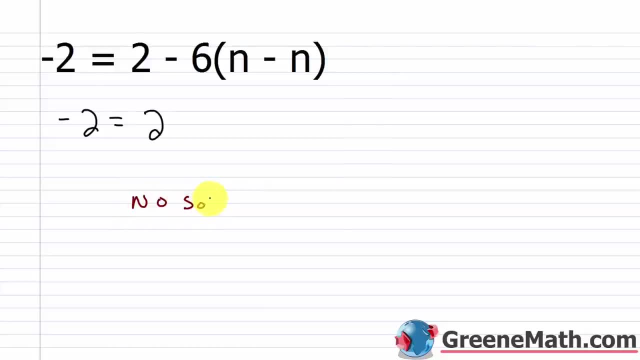 you can put no solution. And again, we'll have some fancy notation for that moving forward. But for right now, just put no solution. Hey, there's nothing I can do here. 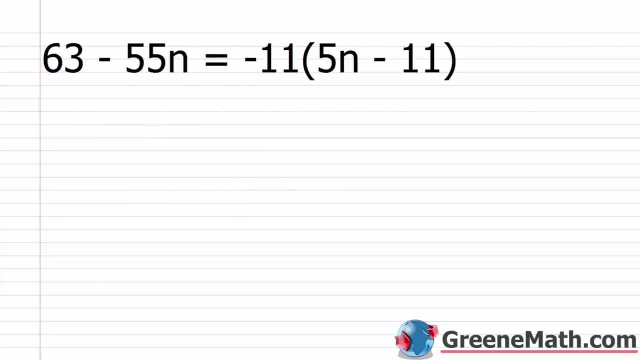 So let's look at some examples and let's see if we can figure out through simplification what type of equation they are. 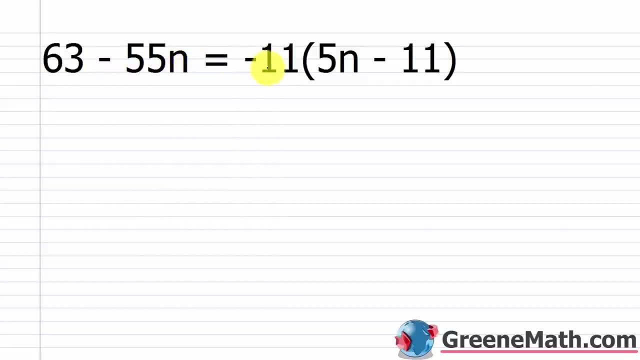 So this one I have 63 minus 55n equals negative 11 times this quantity 5n minus 11. 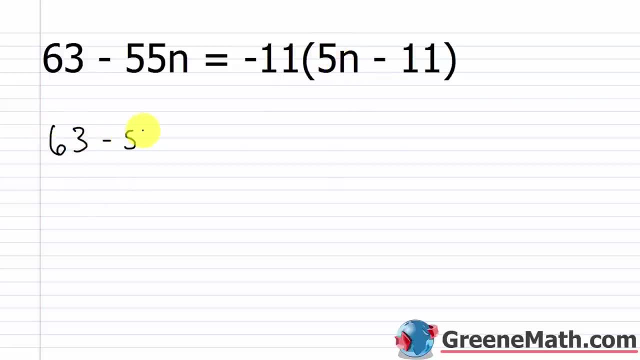 So on the left, 63 minus 55n. On the right, 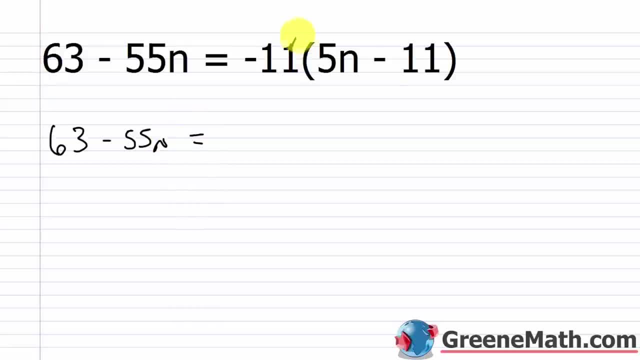 I'm going to use my distributive property to remove the parentheses. So negative 11 times 5n. 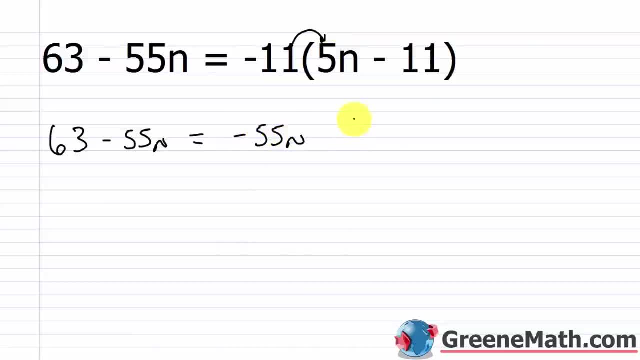 That's negative 55n. And then I'll have negative 11 times negative 11. That's positive 121. 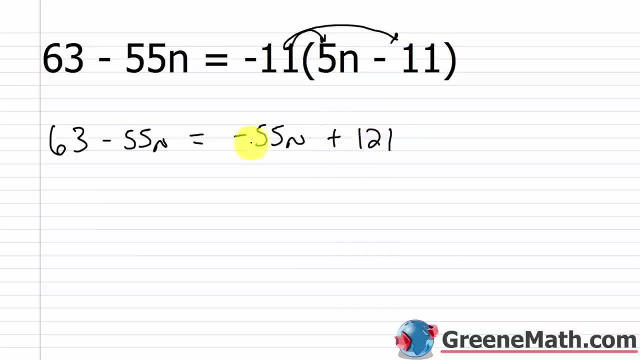 I told you this in one of the videos I made in a previous lesson or practice that I can't remember which one. 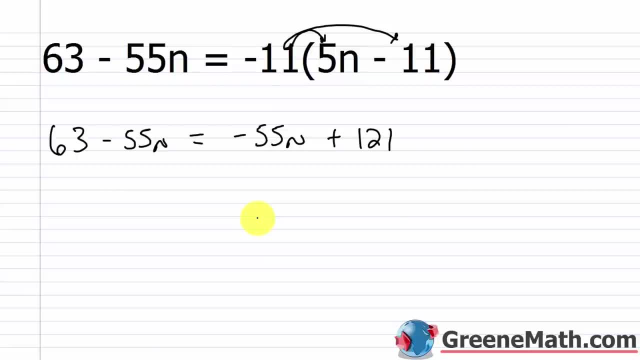 If you have the exact same number on two sides of the equation, you can get rid of it. 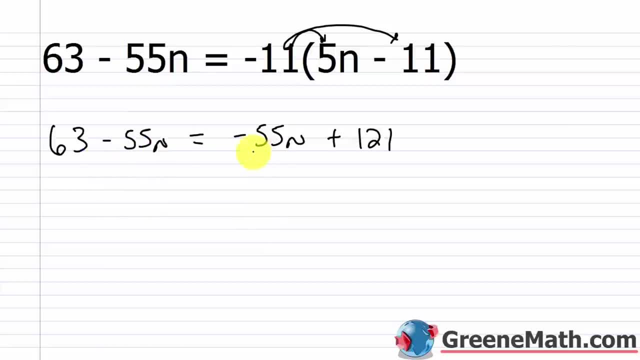 In other words, I have negative 55n here. I have negative 55n here. I can just get rid of it. 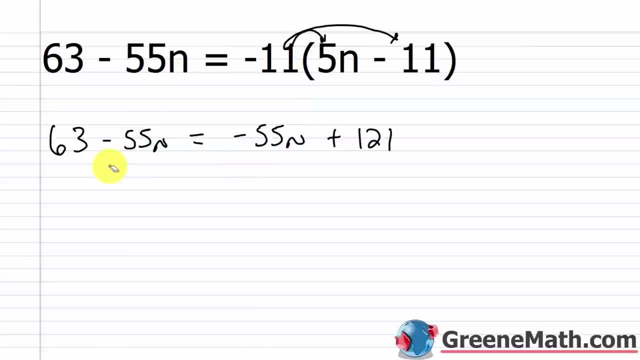 Why is that the case? Well, through the addition property of equality, I can legally make it disappear. 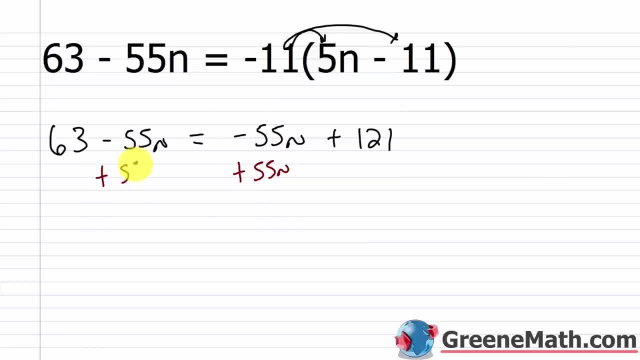 If I add 55n here and I add 55n here, I've added the same number to both sides of the equation. In both cases, it's gone. It sums to zero. 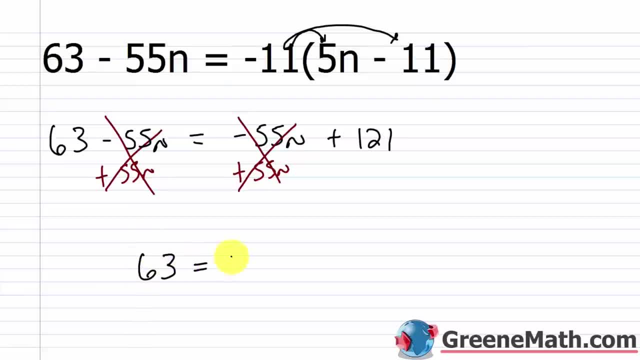 And I'm left with 63 equals 121, which again is nonsense. This is nonsense. Okay, in case you don't know. So there's no solution here. No solution. 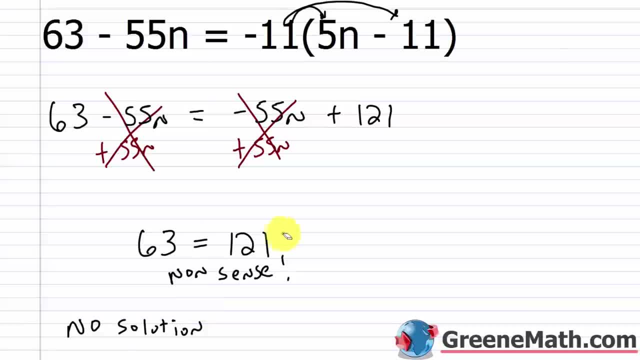 This is another example of a contradiction. If you end up with your variable disappearing and you get one side doesn't equal the other, you have a contradiction. There's not a solution. So this is nonsense. 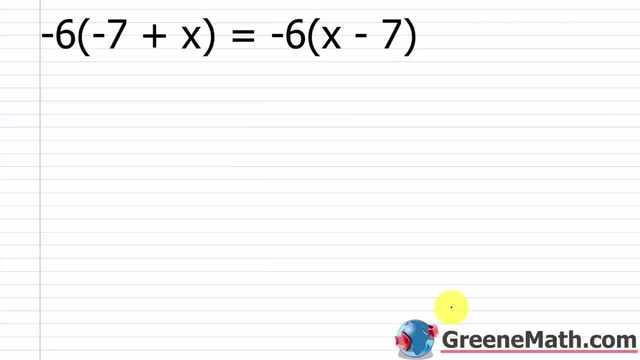 Let's take a look at this one. We have negative 6 times the quantity negative 7 plus x is equal to negative 6 times the quantity x minus 7. 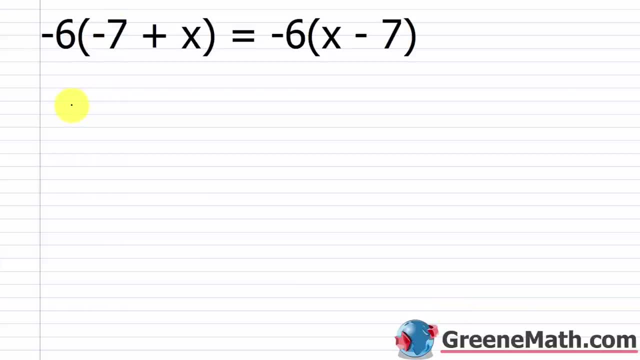 So again, let's simplify. Negative 6 times negative 7 is 42. Negative 6 times x is negative 6x, so minus 6x. Over here, negative 6 times x is negative 6x. 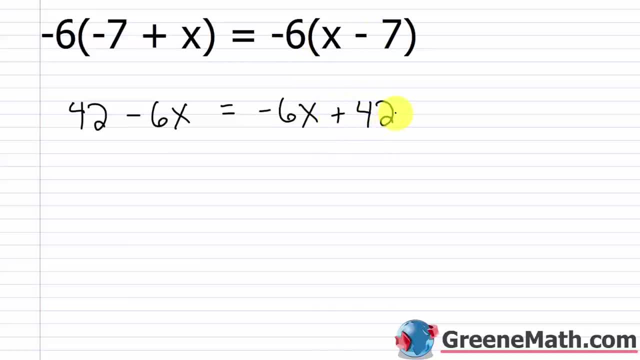 Over here, negative 6 times negative 7 is plus 42. Now if I look closely, 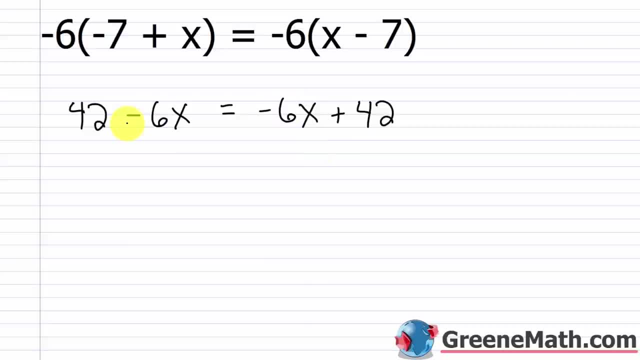 I can see that these are the same. Right? This is an identity. 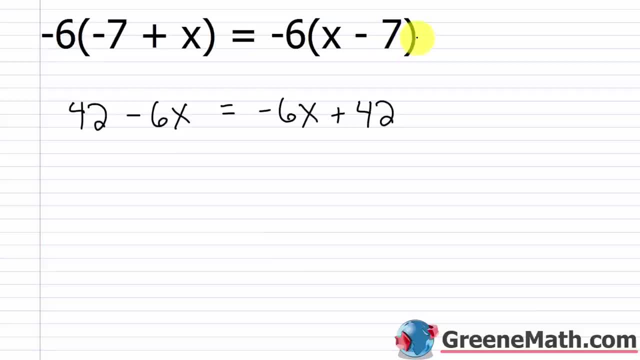 And so upon first glance, and I'm looking at this equation up here, it looks like a regular equation. But once you simplify it and kind of really pay attention, I can reorder this to negative 6x plus 42. 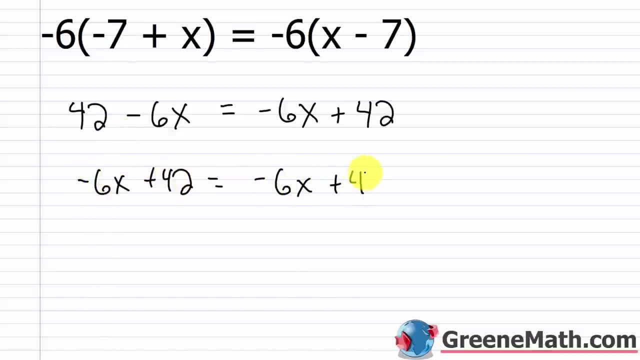 And it's the exact same thing as over here. Negative 6x plus 42. So whatever value I choose for x, doesn't matter what it is, I plug it in, I multiply by negative 6, and I add 42 to it. The same thing is going to happen on both sides of the equation, and so I can pick whatever I want for x, and it'll be a solution. 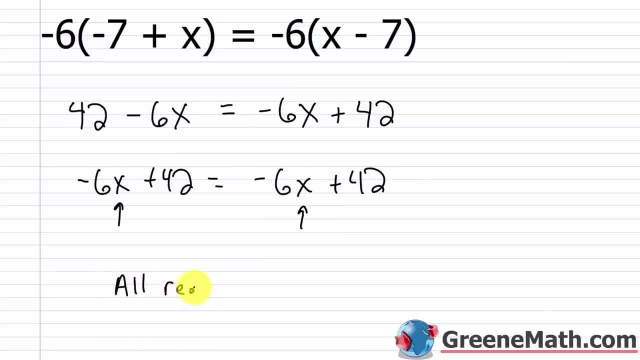 So this would be all real numbers. 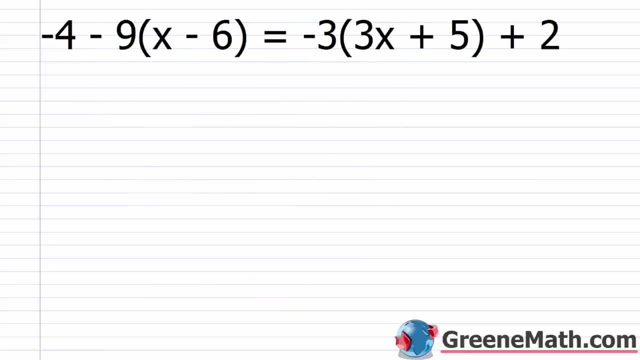 Again, this is an identity. All right, let's take a look at another one. 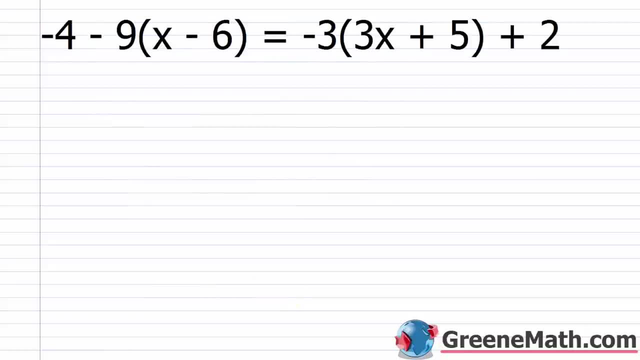 We have negative 4 minus 9 times the quantity x minus 6. This is equal to negative 3 times the quantity 3x plus 5, and then plus 2. 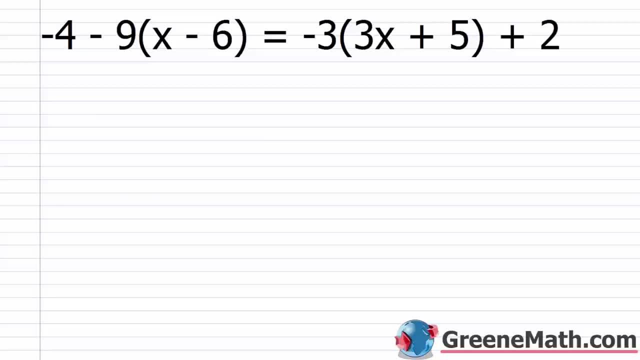 Again, I'm going to simplify each side of the equation, and I'm going to look to see what type of equation I have. 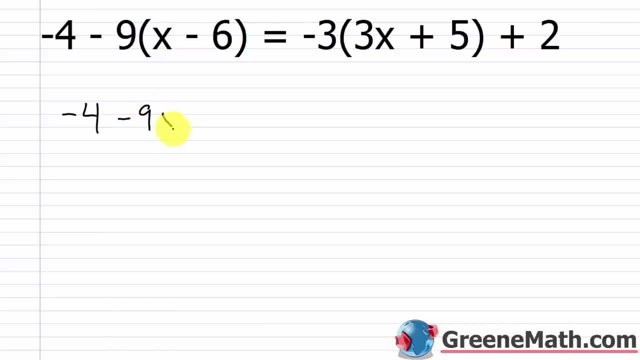 So negative 4, I have negative 9 times x, that's negative 9x, or minus 9x. This is equal to, here I have negative 3 times 3x, that's negative 9x. 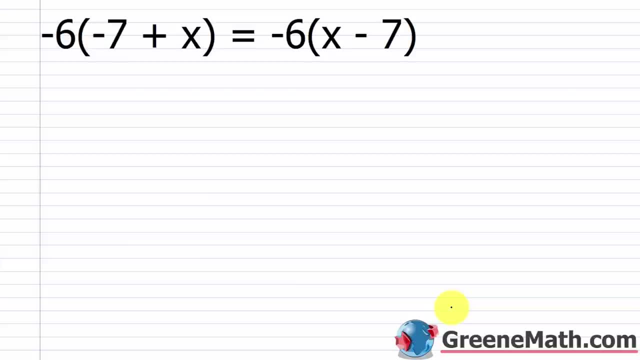 times the quantity X minus seven. So again, let's simplify: Negative six times negative seven is 42.. Negative six times X is negative six X. So minus six X Over here. negative six times X is negative six X Over here. negative six times negative seven is plus 42.. Now, if I look, 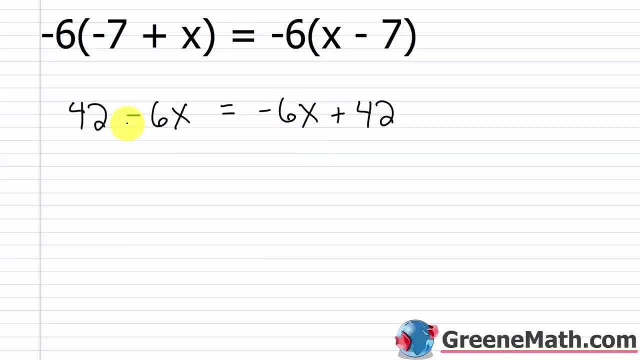 closely, I can see that these are the same right. This is an identity. And so upon first glance- and I'm looking at this equation up here- it looks like a regular equation. But once you simplify it and kind of really pay attention, I can reorder this to negative six X plus 42. And it's the exact. 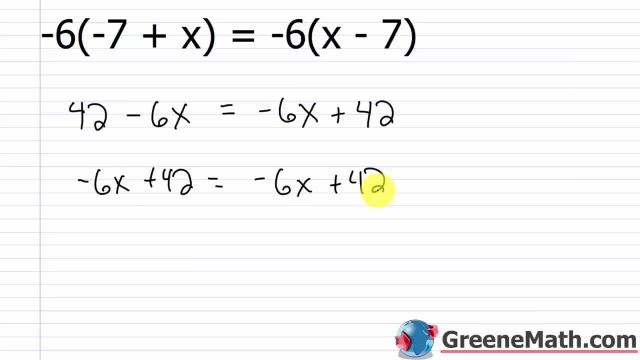 same thing as over here: Negative six, X plus 42. So whatever value I choose for X, doesn't matter what it is. I plug it in, I multiply by negative six and I add 42 to it. The same thing is going to happen on both sides of the equation. 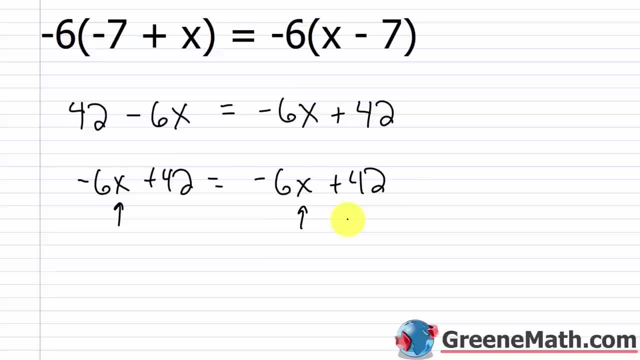 And so I can pick whatever I want for X and it'll be a solution. So this would be all real numbers. Again, this is an identity. All right, let's take a look at another. We have negative four minus nine times the quantity X minus six. This is equal to negative. 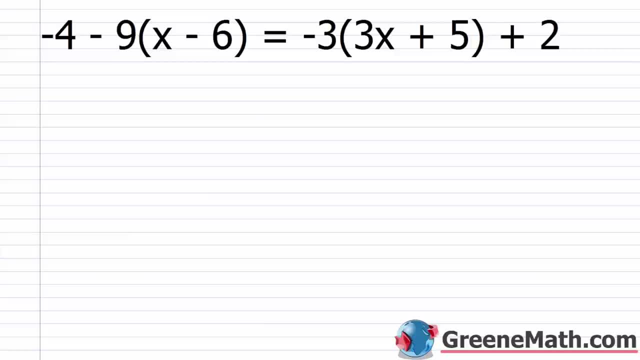 three times the quantity, three X plus five and then plus two Again. I'm going to simplify each one and I'm going to look to see what type of equation I have. So negative four. I have negative nine times X. that's negative. nine X or minus nine X: Negative. nine times negative. six is plus. 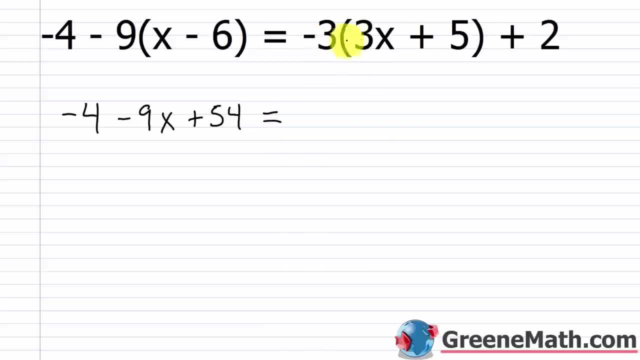 54. This is equal to: here: I have negative three times three, X, that's negative nine X. Then I have negative three times five, that's minus 15, and then plus two. Now, again, again, again. I've told you that if you have the same number on both sides of the equation, 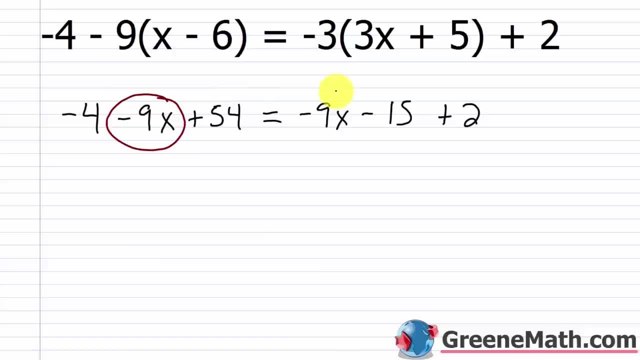 you can get rid of it. So I have negative nine X here. I have negative nine X here. I can cancel them out Again. if I added nine X to both sides of the equation, this is gone. So what am I left with? On the left, negative four plus 54 is 50.. On the right: 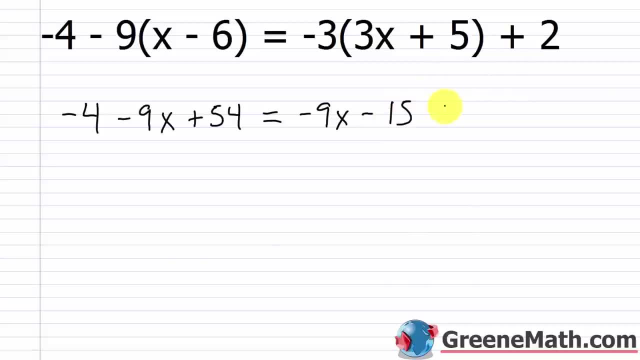 Then I have negative 3 times 5, that's minus 15, and then plus 2. 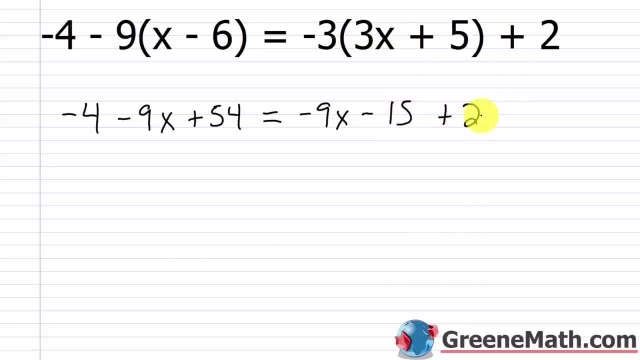 Now, again, again, again, I've told you that if you have the same number on both sides of the equation, you can get rid of it. So I have negative 9x here, I have negative 9x here. I can cancel them out. Again, if I added 9x to both sides of the equation, this is gone. 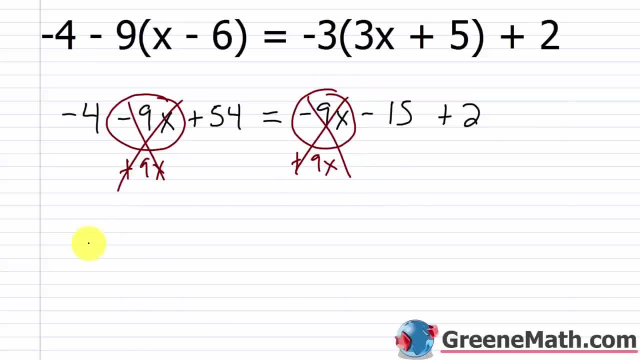 So what am I left with? On the left, negative 4 plus 54 is 50. 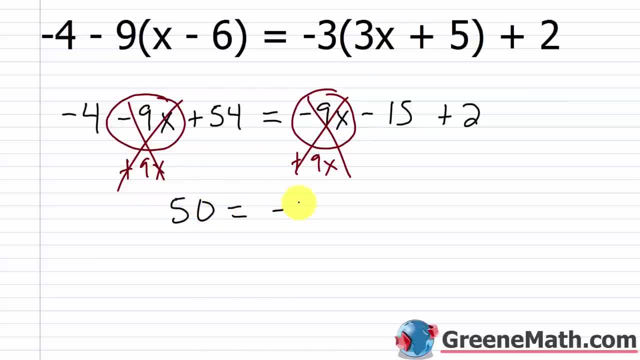 On the right, negative 15 plus 2 is negative 13. 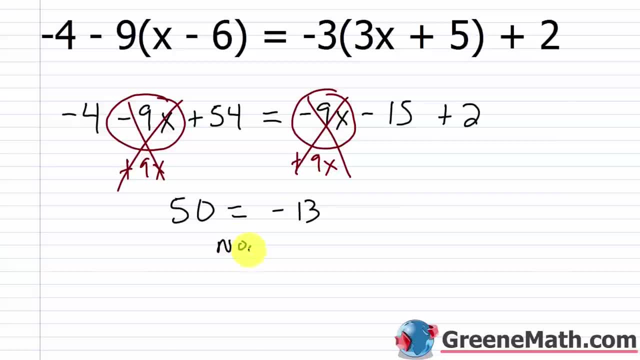 Again, 50 equals negative 13. That's nonsense. Nonsense. Okay? Does not work. So this has no solution. 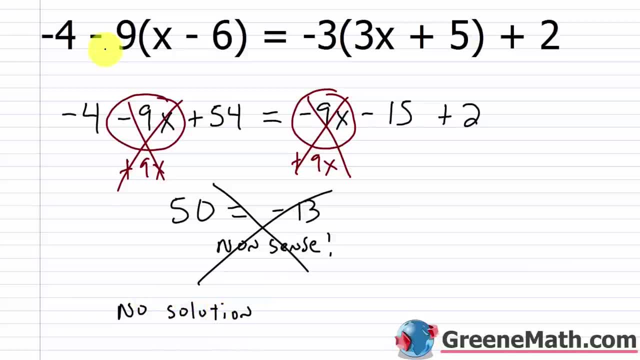 Another example of a contradiction. And again, if you look at this equation to start, it looks like a normal equation, something we would have gotten in previous lessons, right? Something you would just crank out. You're going to get these on a test, usually at the end of the section on linear equations in one variable. 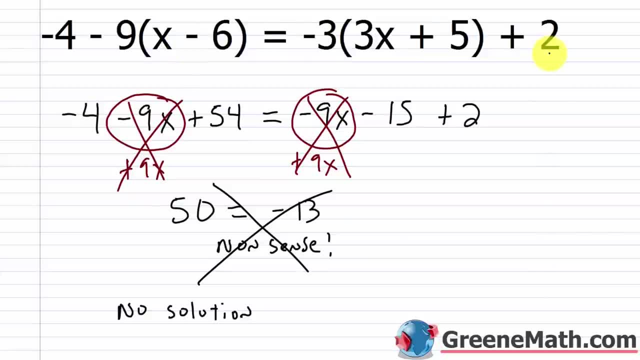 Your teacher is going to throw this at you and expect you to have forgotten about these type of equations. 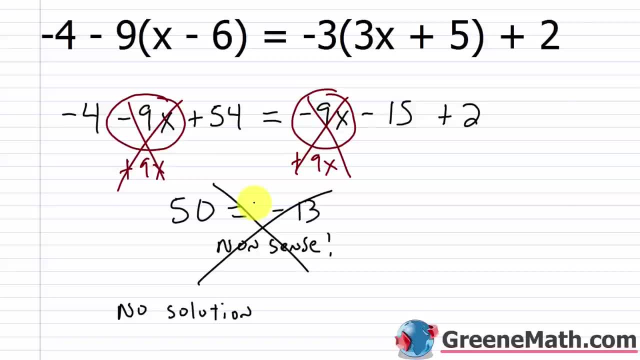 And then you end up trying to solve it and you just, why is the variable gone? 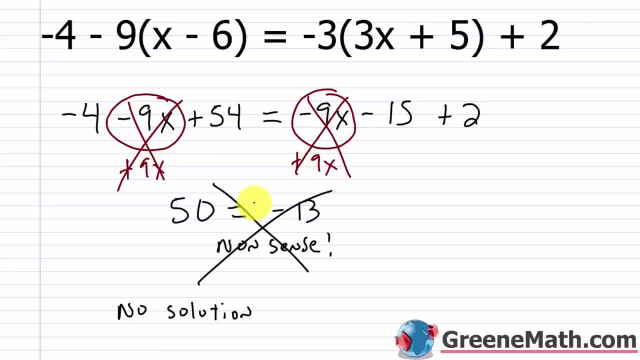 Well, 50 equals negative 13. That doesn't make any sense. So just remember, if the variable is gone and one side doesn't equal the other, there's no solution, right? It's a contradiction. 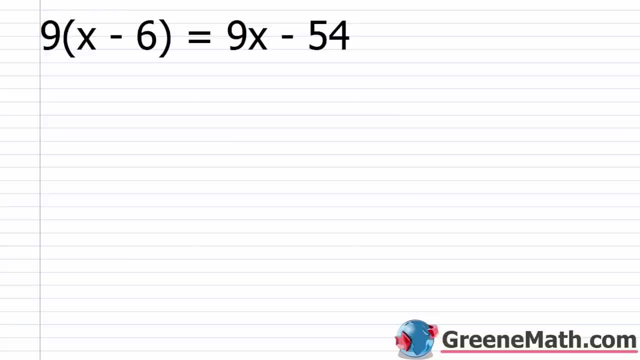 All right. Let's take a look at another example. 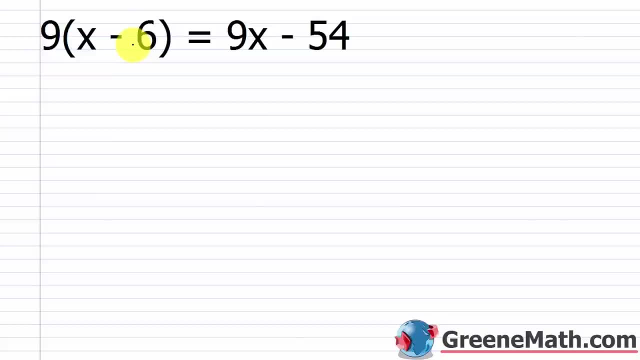 So we have nine times the quantity x minus six equals nine x minus 54. So if I use my distributive property, nine times x is nine x minus nine times six, that's 54. So I have the same thing on the left and the right, nine x minus 54. 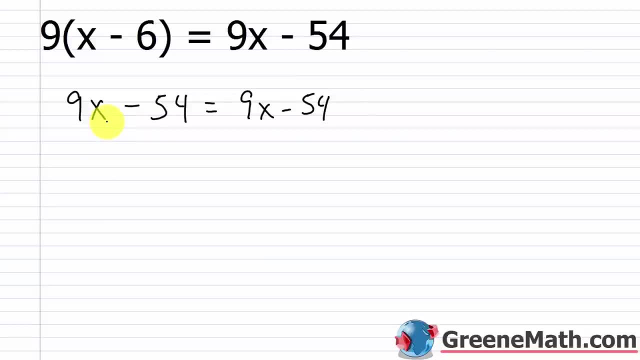 This is an identity, right? I can pick anything for x and it works. So all real numbers, all real numbers would be my solution here. this type of equation is known as an identity. Hello, and welcome to Algebra 1 Lesson 8. 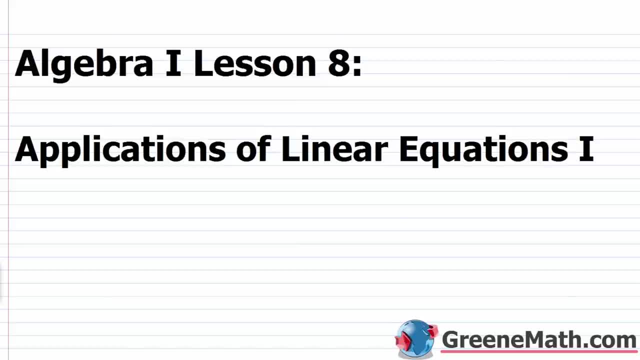 In this video, we're going to talk about applications of linear equations. 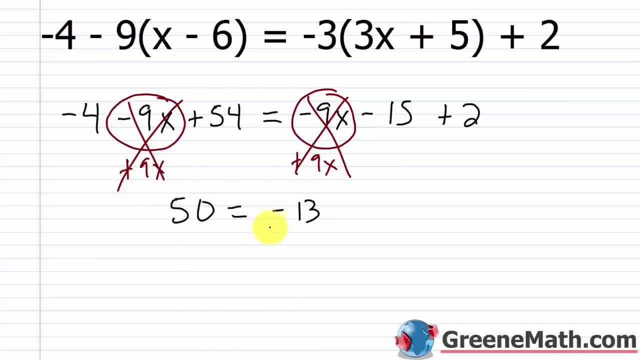 negative. 15 plus two is negative 13.. Again, 50 equals negative 13.. That's nonsense. Nonsense, okay, Does not work. This has no solution. Another example of a contradiction, And again, if you look at this, 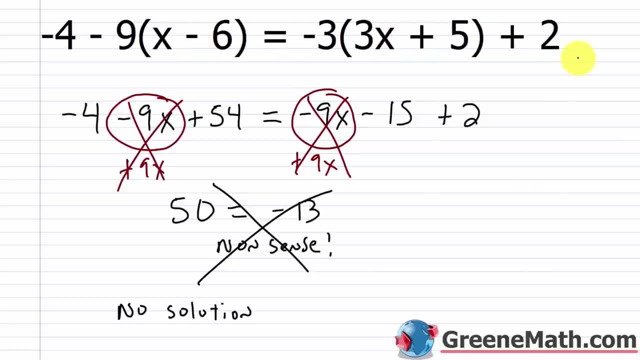 equation. to start, it looks like a normal equation, something we would have gotten in previous lessons, right? Something you would just crank out. You're going to get these on a test, usually at the end of the section on linear equations in one variable. Your teacher is going. 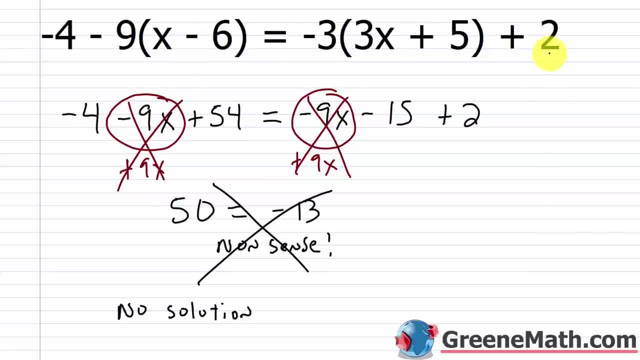 to throw this at you and expect you to have forgotten about these type of equations. And then you end up trying to solve it And you just, why is the Why is the variable gone? Well, 50 equals negative 13.. That doesn't make any sense, So just. 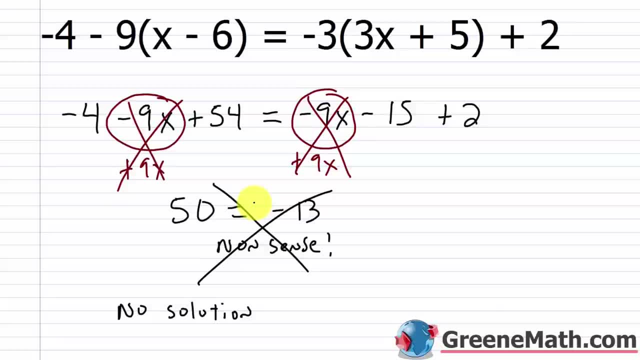 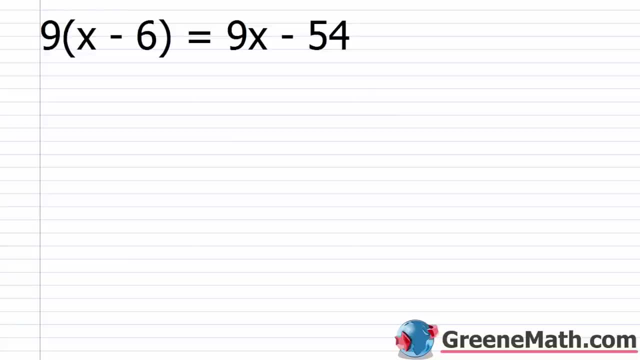 remember, if the variable is gone and one side doesn't equal the other, there's no solution, right? It's a contradiction. All right, let's take a look at another example. So we have nine times the quantity X minus six equals nine X minus 54.. So if I use my distributive property, 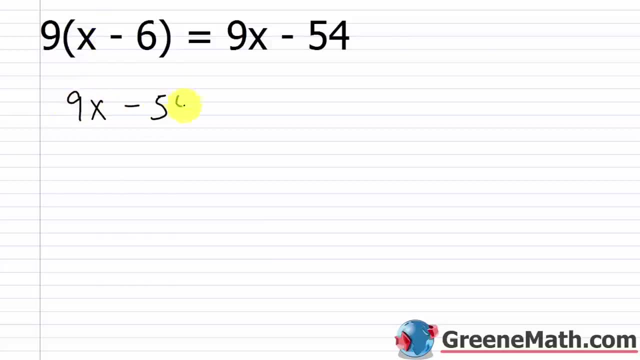 nine times X is nine. X minus nine times six, that's 54. So I have the same thing on the left and the right: nine X minus 54. This is an identity right. I can pick anything for X and it works. So all real numbers. 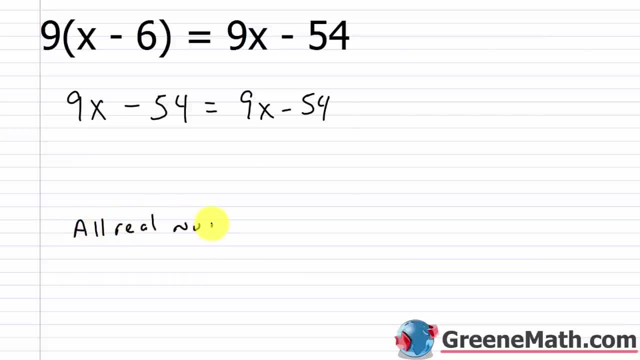 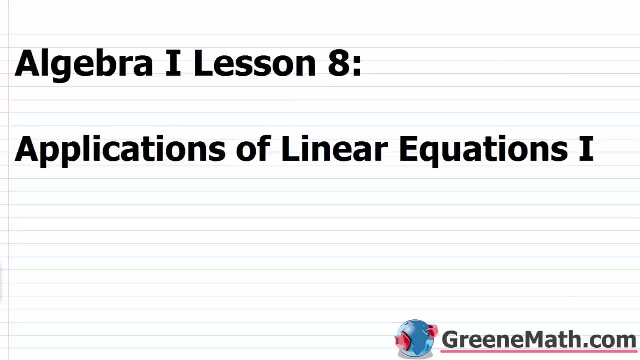 all real numbers would be my solution here And again. this type of equation is known as an identity. Hello and welcome to Algebra 1, Lesson 8.. In this video, we're going to talk about applications of linear equations. This is going to be the first section of that. 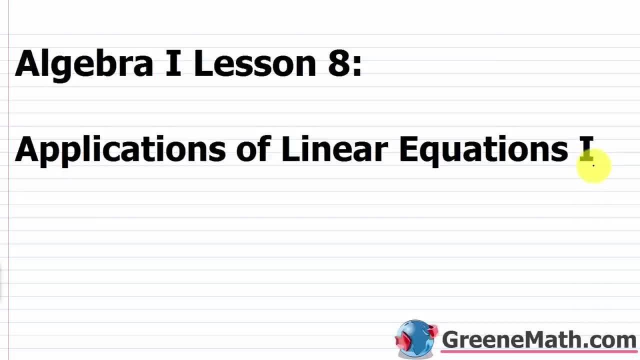 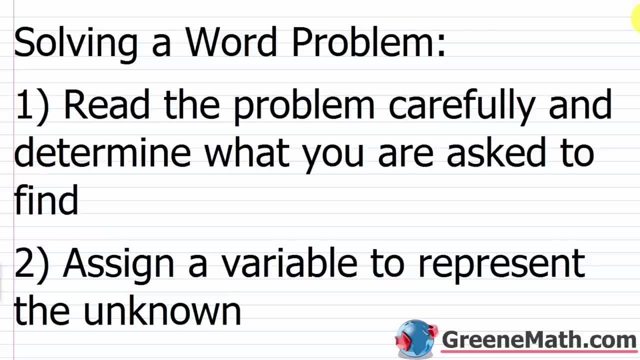 And a lot of you will know this as solving word problems. Before we kind of get started, I just want to tell you that once you've mastered the material that we've presented in the first seven sections of this course, you're ready to move on and start. 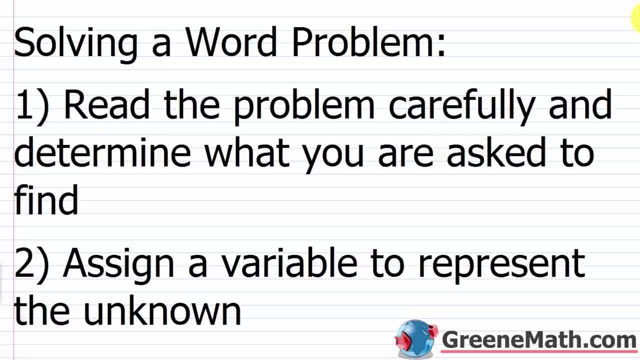 solving word problems. Now, this is where a lot of students really get frustrated. When you start solving word problems, it's unlike solving the problems you've gotten before. Now, in addition to solving an equation, you also have to figure out how to get the equation. So that's what makes 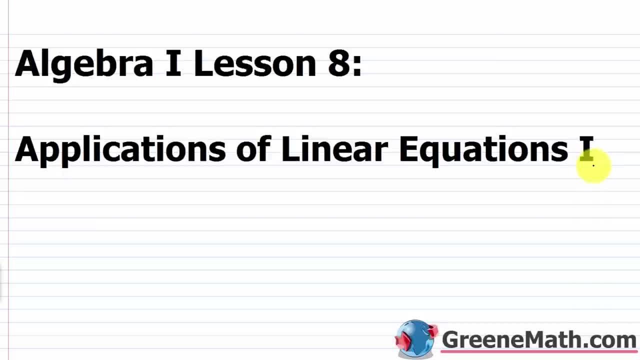 This is going to be the first section of that. And a lot of you will know this as solving word problems. 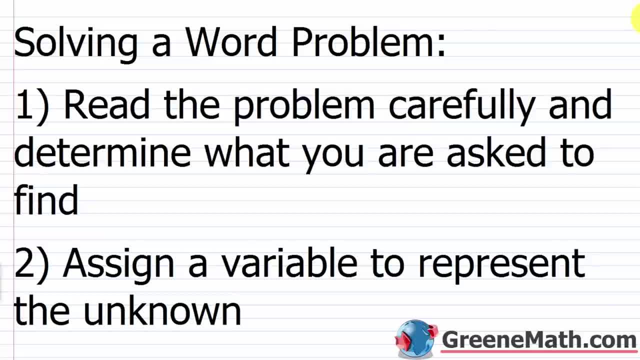 So before we kind of get started, I just want to tell you that once you've mastered the material 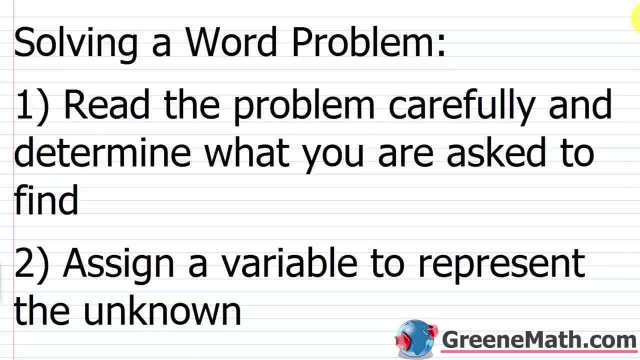 that we've presented in the first seven sections of this course, you're ready to move on and start solving word problems. 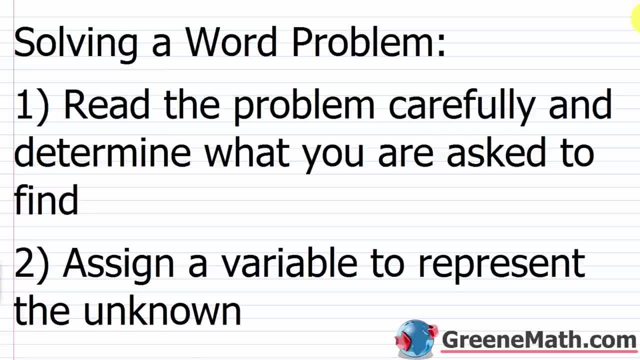 Now, this is where a lot of students really get frustrated. 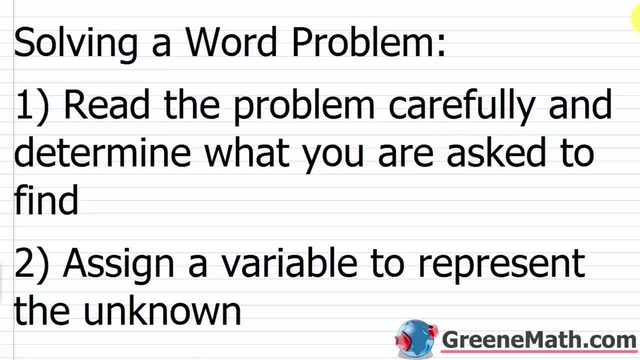 When you start solving word problems, it's unlike solving the problems you've gotten before. Now, in addition to solving an equation, 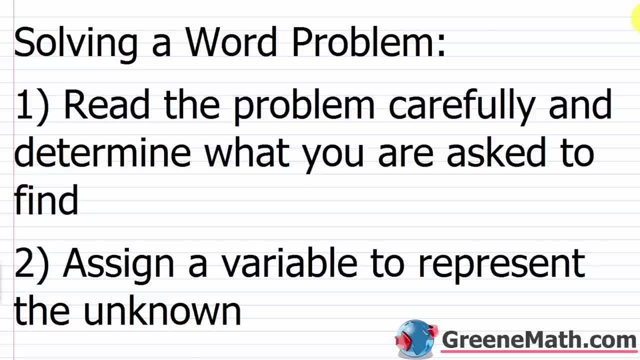 you also have to figure out how to get the equation. So that's what makes word problems so difficult. 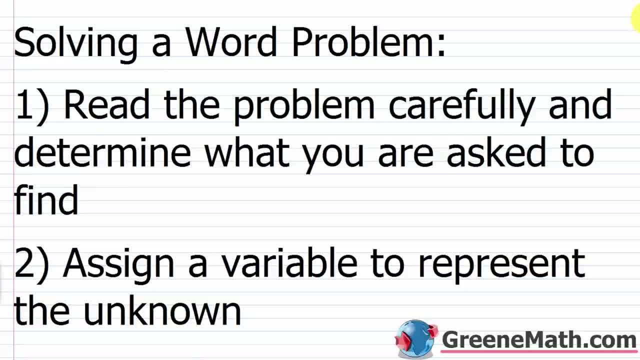 You have to read through and figure out your own equation before you even solve it. 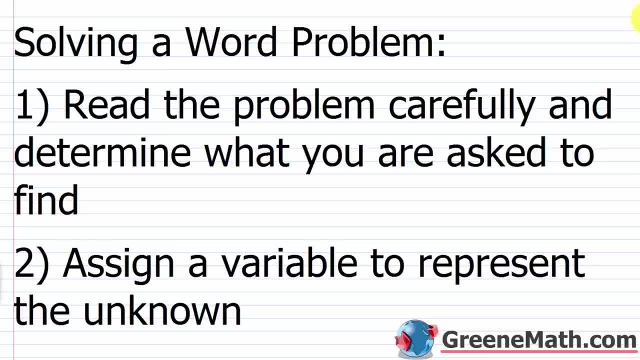 So the first thing I want to do here is I want to go through a brief procedure that we can use when we're solving a word problem. Now, your textbook might have something that's different. If you want to follow that, do so. If you want to follow mine, do so. If you want to follow your teachers, do so. 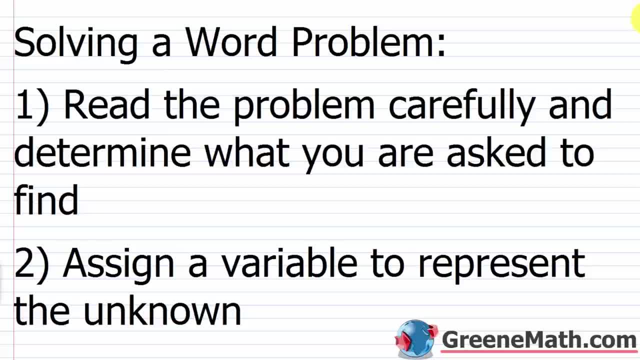 The main goal here is to get a procedure that you can follow each and every time until you feel completely comfortable with word problems. All right, so solving a word problem. 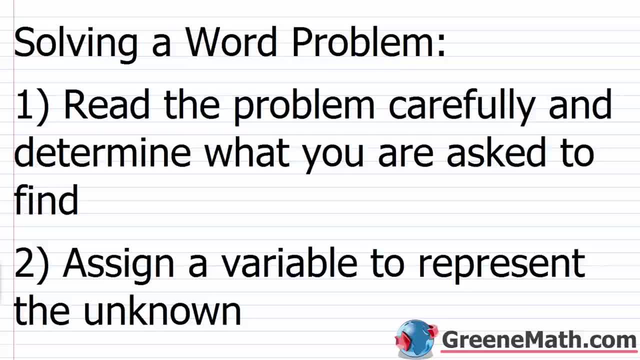 So the first thing and probably the most important thing is to read the problem carefully and determine what you are asked to find. 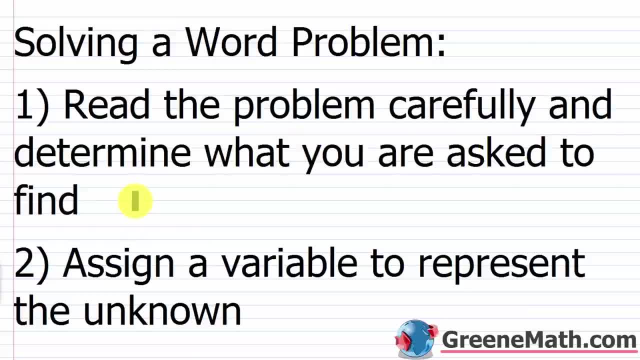 I can't tell you how many students I've tutored and, you know, 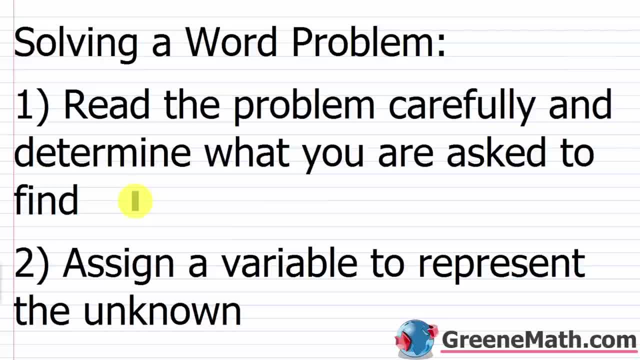 we do a sample problem and they don't even know what they're looking for. So this is probably the most important thing. 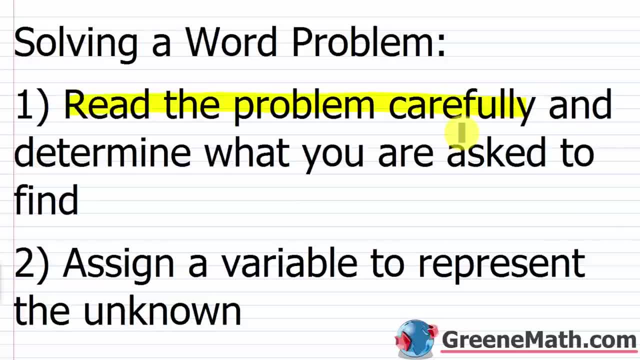 Just to read the problem carefully again and determine what you are asked to find. 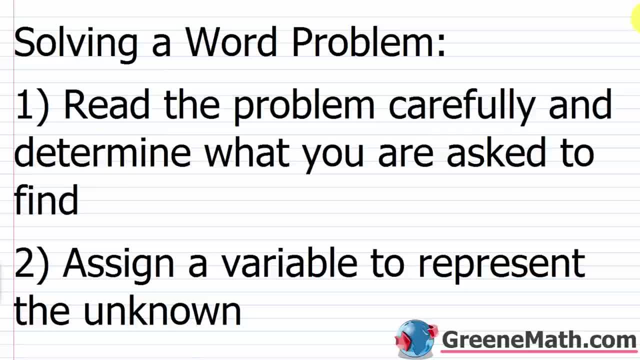 word problems so difficult, You have to read through the equation and figure out how to get the equation. So the first thing I want to do here is I want to go through a brief procedure that we can use when we're solving a word problem. Now your textbook might have something that's. 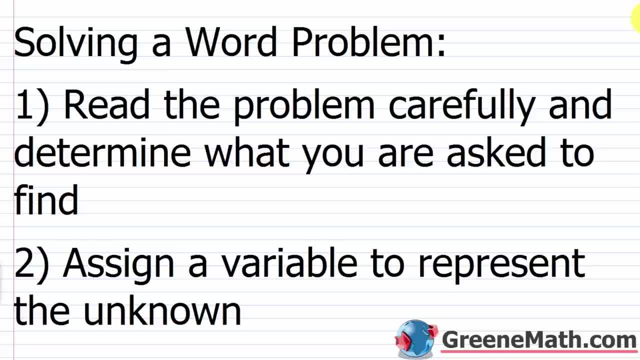 different. If you want to follow that, do so. If you want to follow mine, do so. If you want to follow your teachers, do so. The main goal here is to get a procedure that you can follow each and every time until you feel completely comfortable with word problems. 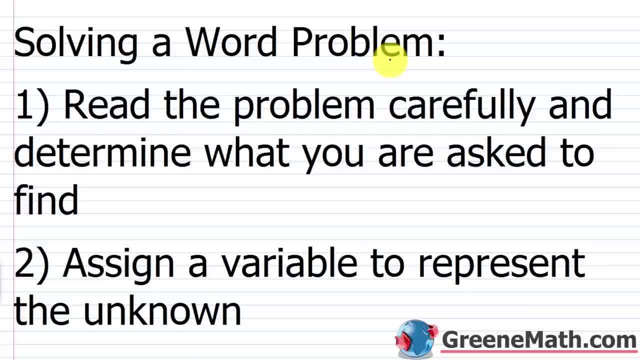 Alright, so solving a word problem. So the first thing, and probably the most important thing, is to read the problem carefully and determine what you are asked to find. I can't tell you how many students I've tutored, and you know we do a sample problem and they don't even know what. 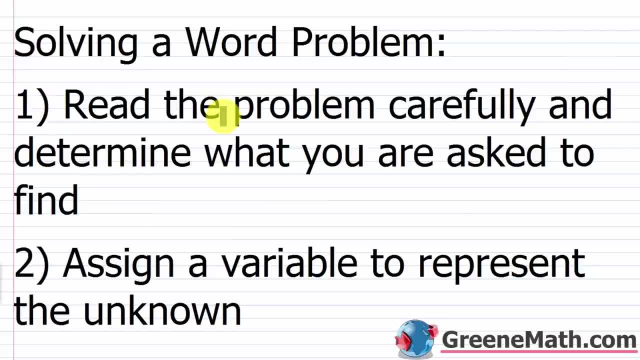 they're looking for. So this is probably the most important thing: Just to read the problem carefully again and determine what you are asked to find. I always make my tutoring students write out: hey, this is what I'm looking for, so that they know what the overall goal is. 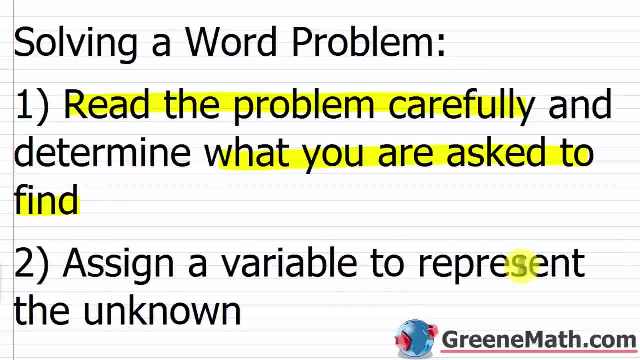 Alright. now the next thing is to assign a variable to represent the unknown. Sometimes there's going to be more than one unknown and as we get through algebra you're going to have a lot more complicated scenarios than you're going to face when you're just working with linear equations. 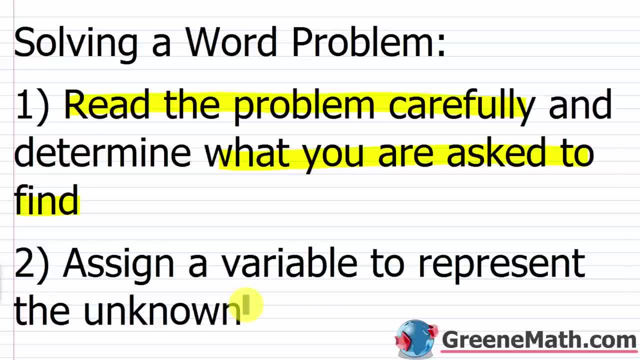 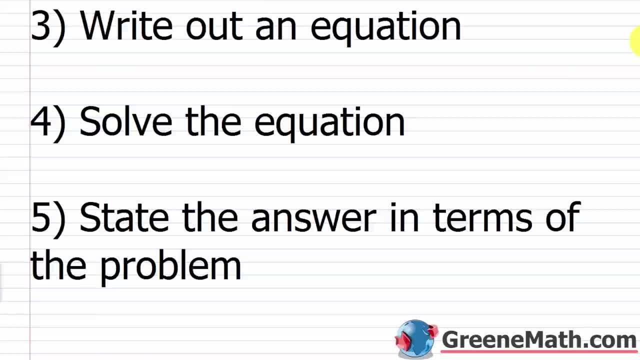 in one variable For the problems we're going to look at here. if we have two unknowns, we're going to be able to represent one of the unknowns in terms of the variable. So this is going to be one of the unknowns in terms of the other, Alright. so the next thing we're going to do is we're 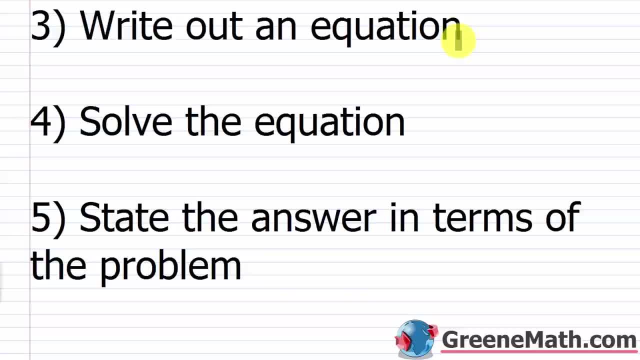 going to write out an equation And the way we do that, we read back through our problem and we're going to see that something is equal to something else. They're always going to give you a way to set up an equation so that you can get an answer. Now we get to the easy part. We just solve the. 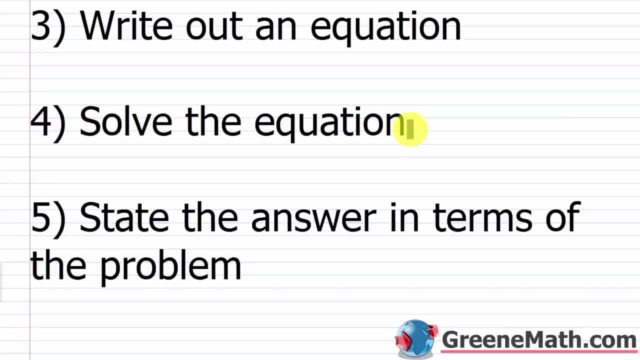 equation. So this is the part that we already know how to do. Then, part five, we state the answer in terms of the problem. So, in regards to a word problem, that's generally going to be a nice little sentence describing your answer. Then last thing we're going to do is we're going to 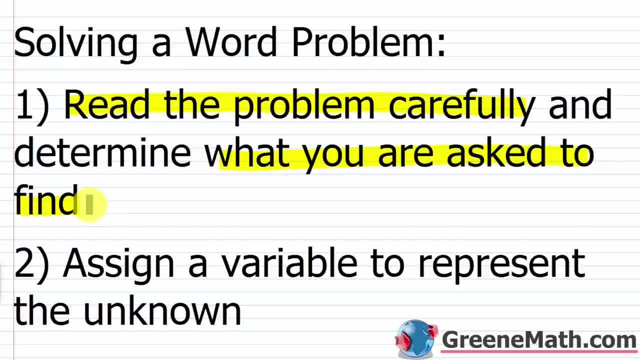 I always make my tutoring students write out. Hey, this is what I'm looking for so that they know what the overall goal is. All right. 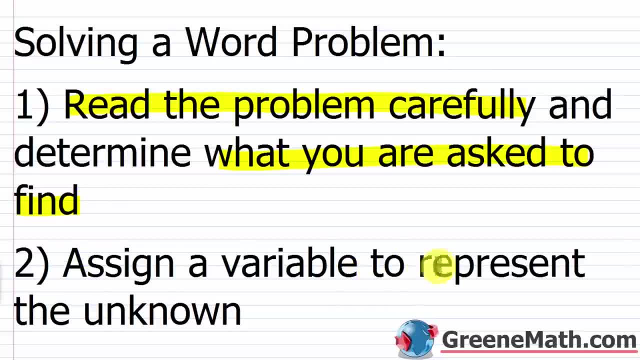 Now, the next thing is to assign a variable to represent the unknown. 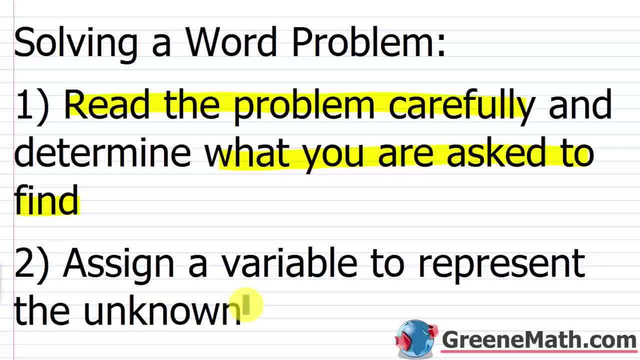 Sometimes there's going to be more than one unknown. And as we get through algebra, 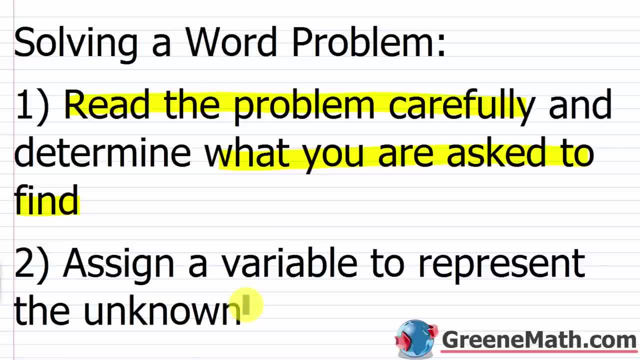 you're going to have a lot more complicated scenarios than you're going to face when you're just working with linear equations in one variable. 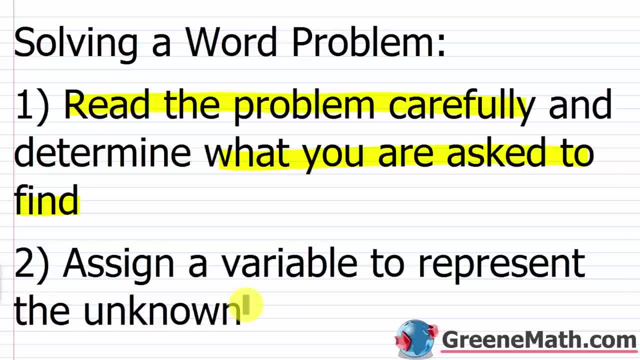 For the problems we're going to look at here, if we have two unknowns, we're going to be able to represent one of the unknowns in terms of the other. 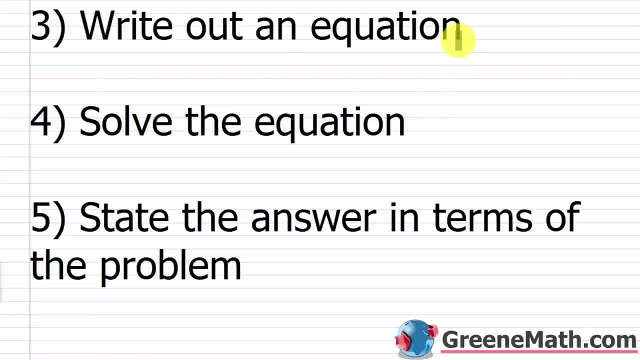 All right, so the next thing we're going to do is we're going to write out an equation. And the way we do that, we're going to go through our problem and we're going to see that something is equal to something else. 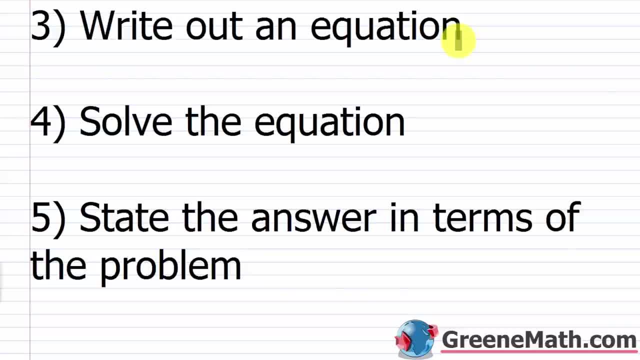 They're always going to give you a way to set up an equation so that you can get an answer. 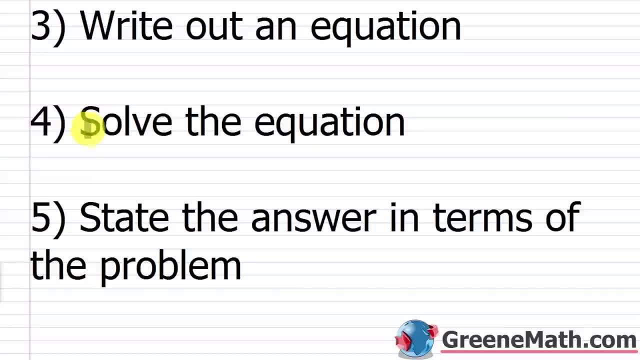 Now we get to the easy part. We just solve the equation. So this is the part that we already know how to do. Then part five, 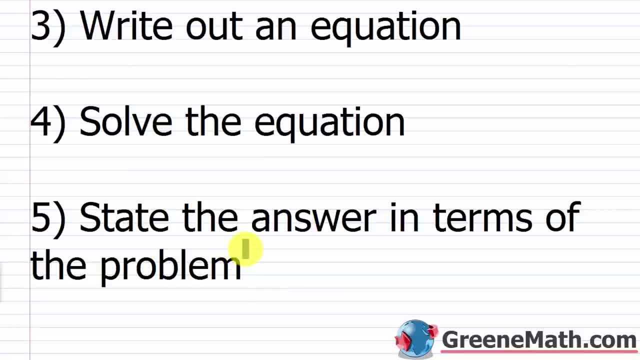 we state the answer in terms of the problem. So in regards to a word problem, that's generally going to be a nice little sentence describing your answer. 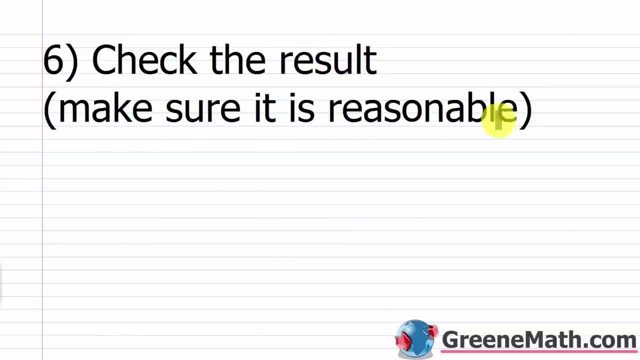 Then lastly, we want to check the result and make sure it's reasonable. 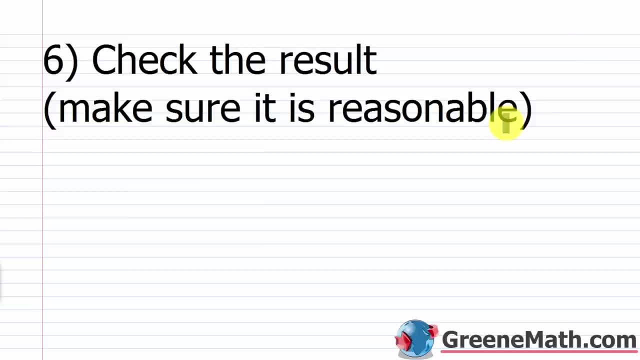 So for example, if you're asked how many people are on a train and you get an answer of 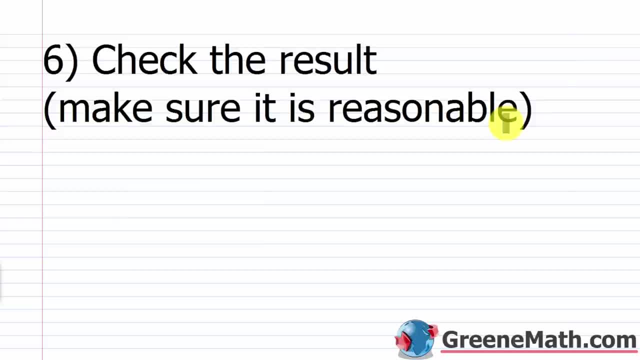 24.65, you're probably wrong, right? Because there's not 0.65 of a person. 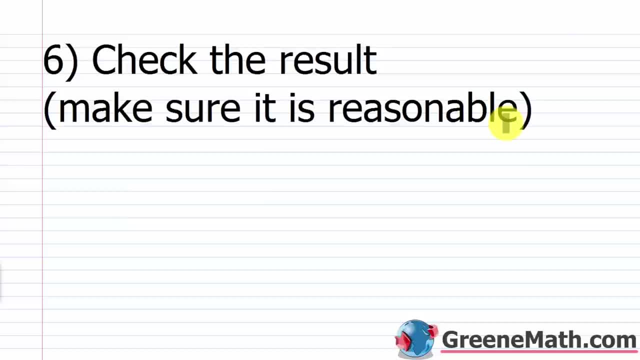 So you're looking for a nice whole number, or let's say they ask how many people are on a train and you get negative seven. 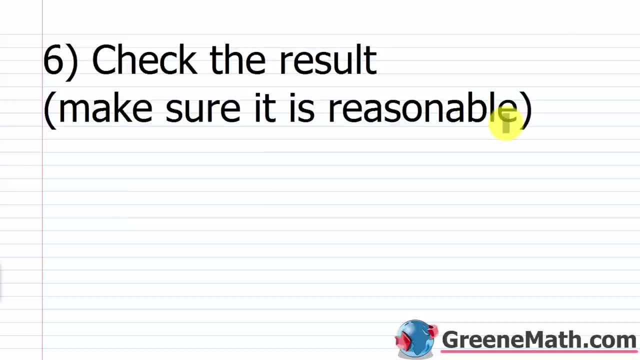 That doesn't make any sense. So when you're solving word problems, 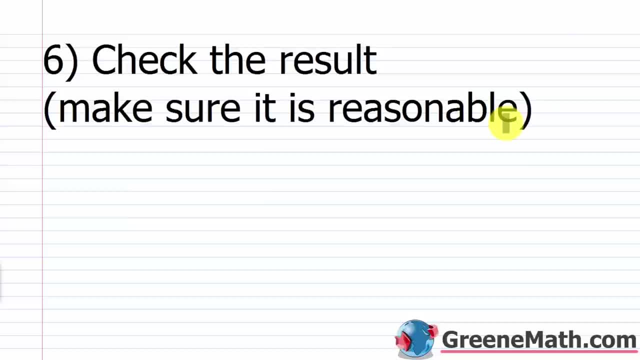 you need to make sure that your answer is reasonable. If it's not, you probably made a mistake. 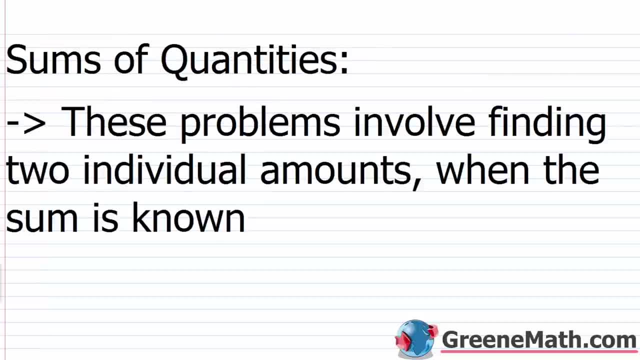 All right, so let's start out by looking at some different types of problems that you might encounter. The first type is called sums of quantities. 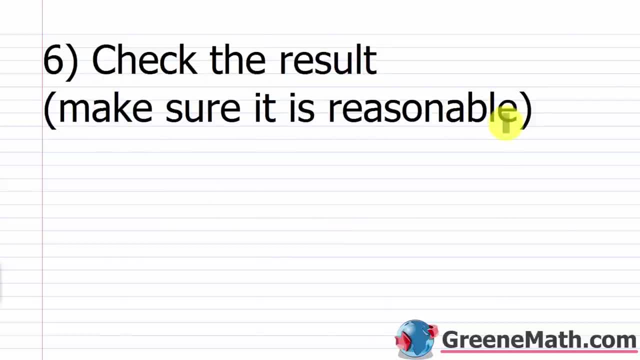 check the result and make sure it's reasonable. So, for example, if you're asked how many people are on a train and you get an answer of 24.65, you're probably wrong. right, Because there's not 0.65 of. 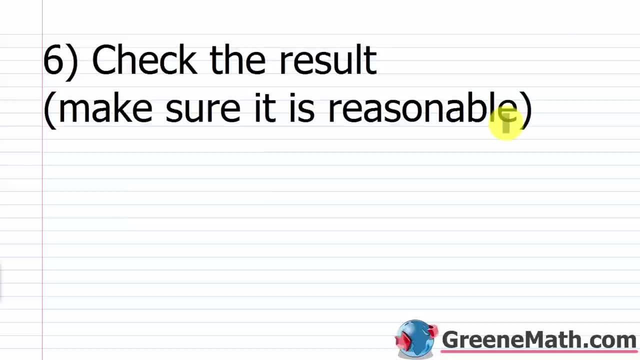 a person. So you're looking for a nice whole number. Or let's say, they ask how many people are on a train and you get negative seven. That doesn't make any sense. So when you're solving word problems, you need to make sure that your answer is reasonable. If it's not, you probably 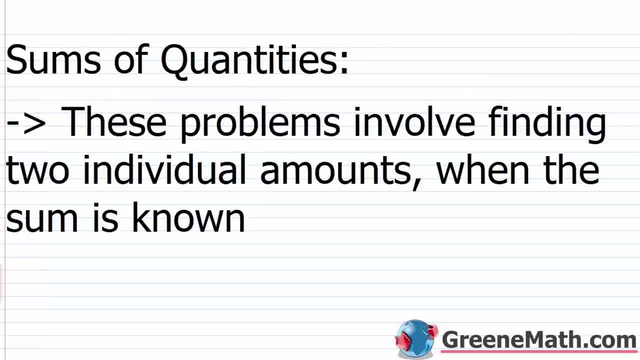 made a mistake. Alright, so let's start out by looking at the answer. So let's start out by looking at some different types of problems that you will encounter. The first type is called sums of quantities, So you're going to see these right away when you get to your algebra one. 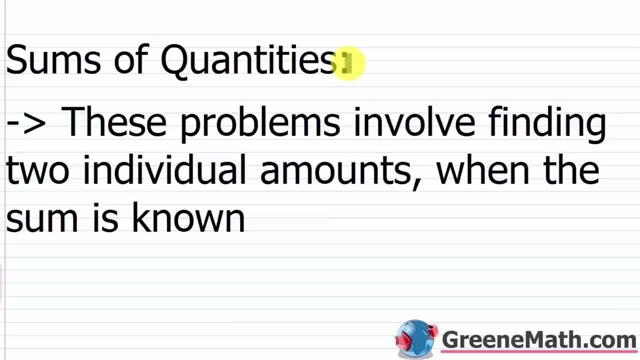 section on applications of linear equations, And these problems involve finding two individual amounts- sometimes it's more than two- when the sum is known. So that's the key. So you're finding individual amounts when the sum is known. So let's take a look at an example. So the phantoms one. 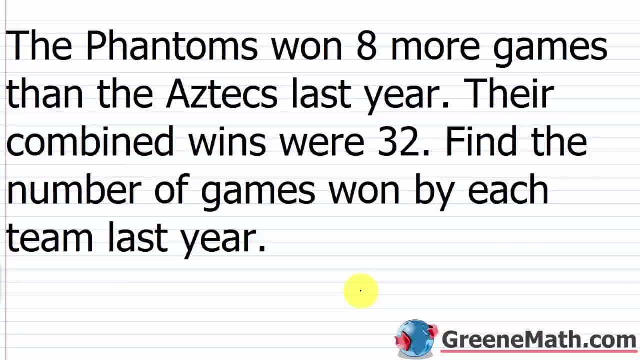 eight more games than the Aztecs last year. Their combined wins were 32.. Find the number of games won by each team last year. So kind of. our first step is to read the problem and determine what you're asked to find. So we've read the problem. I recommend reading it more than once and writing. 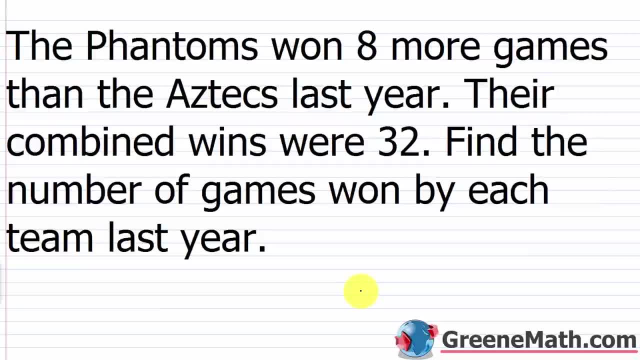 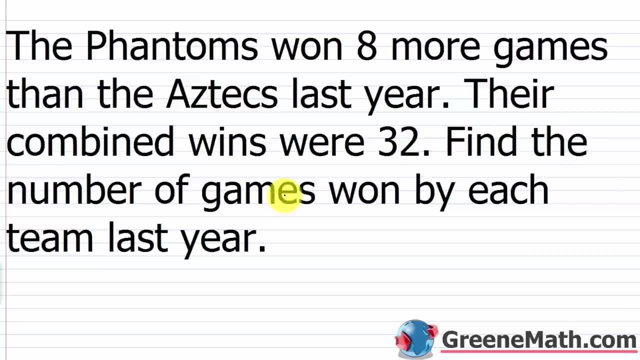 year. Their combined wins were 32.. Find the number of games won by each team last year. So this is my goal: I want to find the number of games won by each team last year. So at the end of the day, I'm. 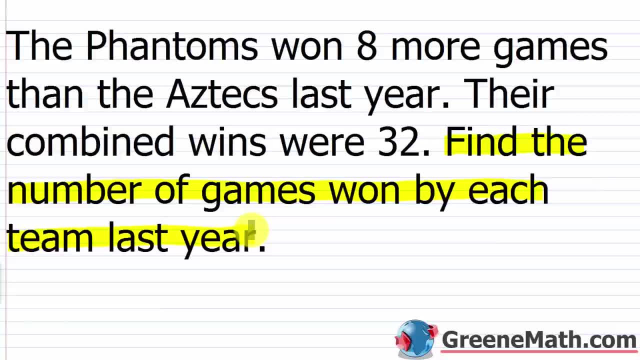 going to be writing a nice little sentence saying that the Aztecs won this many games and the phantoms one this many games, based on the information given in the problem. Alright, so now we're going to move on to the next step. 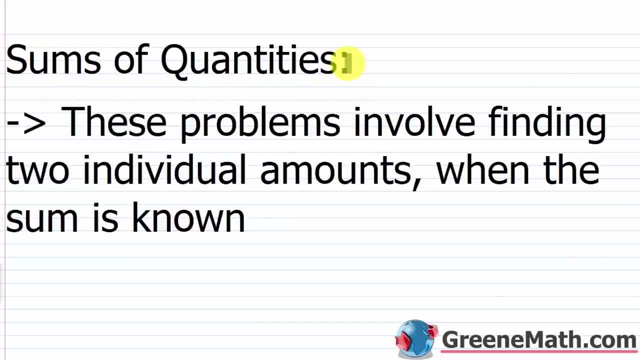 So you're going to see these right away when you get to your algebra one section on applications of linear equations. And these problems involve finding two individual amounts. 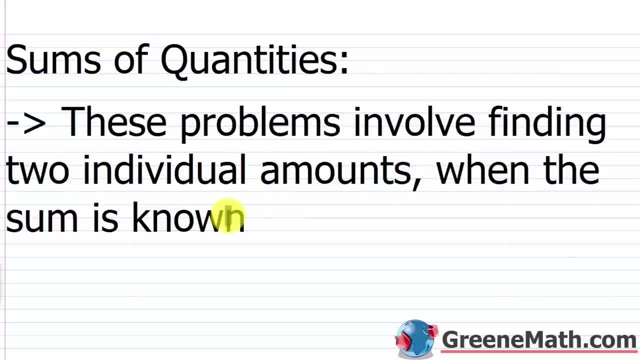 Sometimes it's more than two when the sum is known. So that's the key. 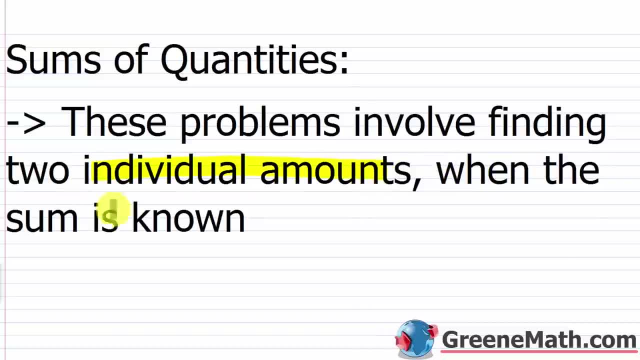 So you're finding individual amounts when the sum is known. 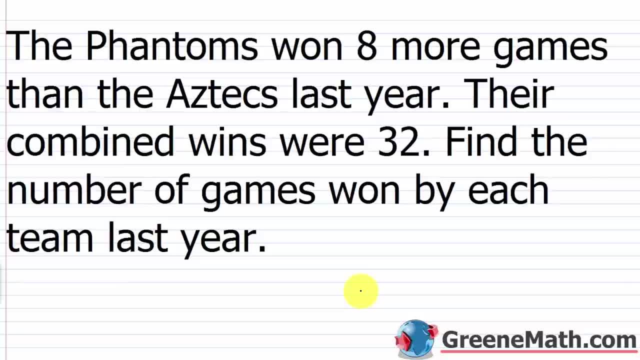 So let's take a look at an example. So the phantoms won eight more games than the Aztecs last year. Their combined wins were 32. 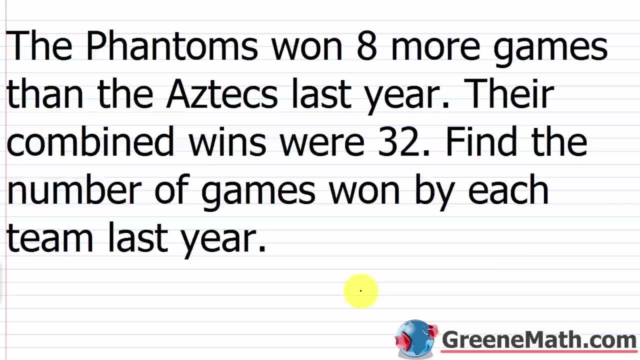 Find the number of games won by each team last year. So kind of our first step is to read the problem and determine what you're 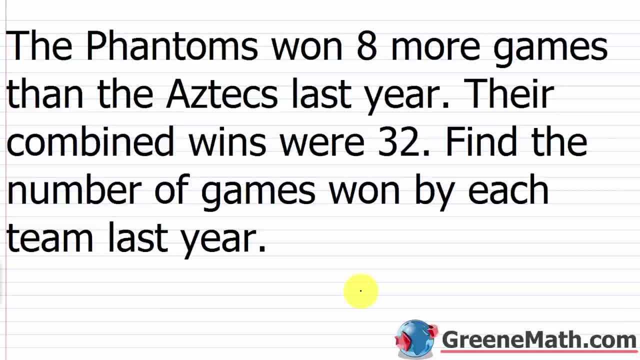 asked to find. So we've read the problem. I recommend reading it more than once and writing down specifically what your goal is. That way you're going to have a laser focus. So again, the phantoms won eight more games than the Aztecs last year. 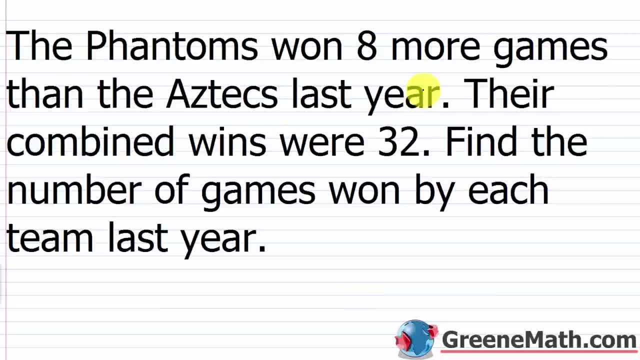 Their combined wins were 32. So again, their combined wins were 32. 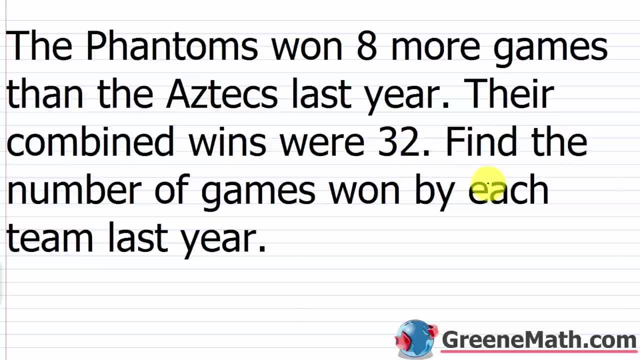 Find the number of games won by each team last year. So this is my goal. I want to find the number of games won by each team last year. 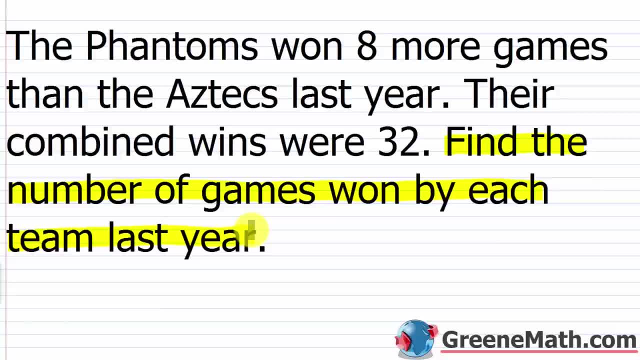 So at the end of the day, I'm going to be writing a nice little sentence saying that the Aztecs won this many games and the phantoms won this many games based on the information given in the problem. 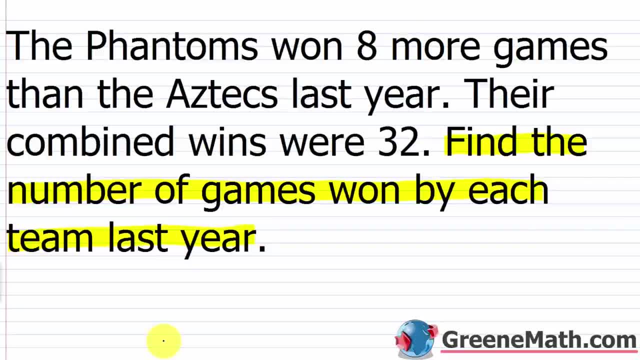 All right, so now we're going to move on to the next step and this step is a little bit challenging for students. So I want you to pay close attention. 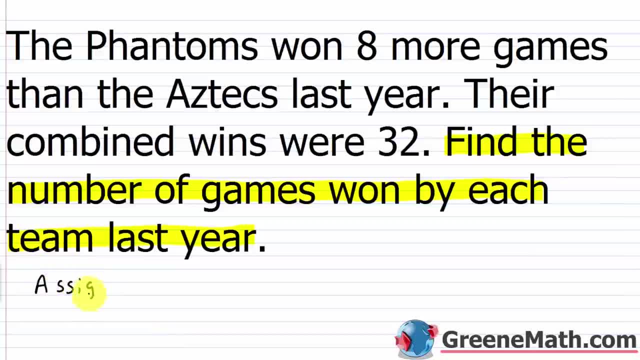 So this step is assign a variable. So how do we assign a variable? What do we do? Well, remember we're assigning a variable to represent the unknown. 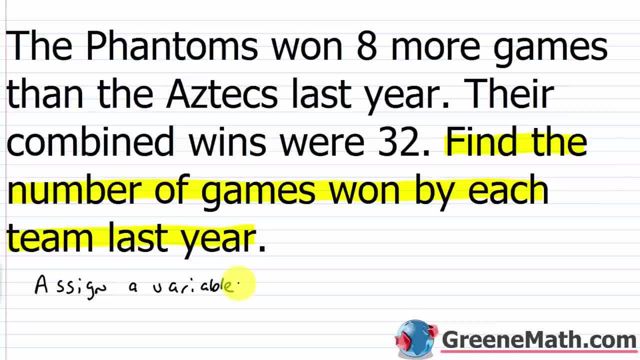 In this case, we have two unknowns and our two unknowns would be how many games. So how many games did the Aztecs win? 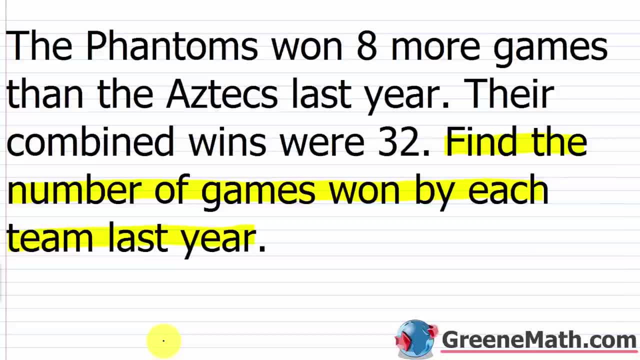 And this step is a little bit challenging for students, So I want you to pay close attention. So this step is: assign a variable. So how do we assign a variable? What do we do? Well, remember, we're assigning a variable to represent the unknown. 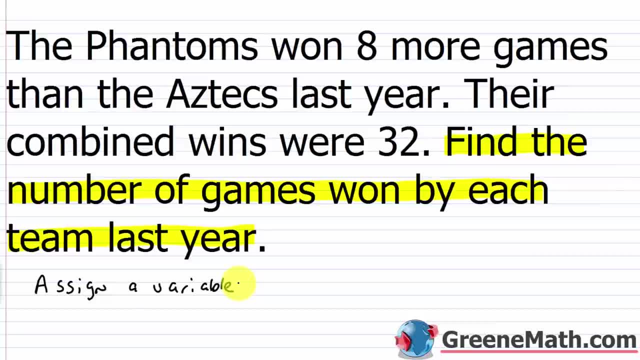 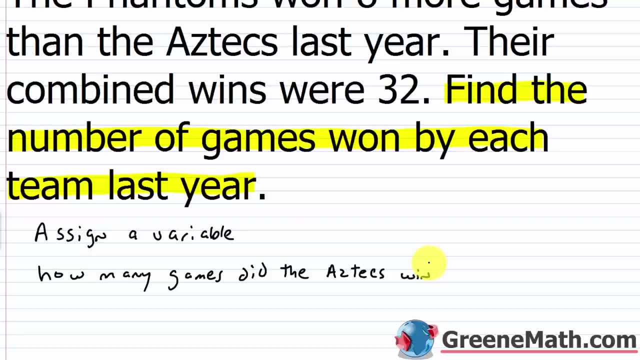 In this case, we have two unknowns, And our two unknowns would be: how many games? So how many games did the Aztecs win? And then also, how many games did the Phantoms win? These are our two unknowns. 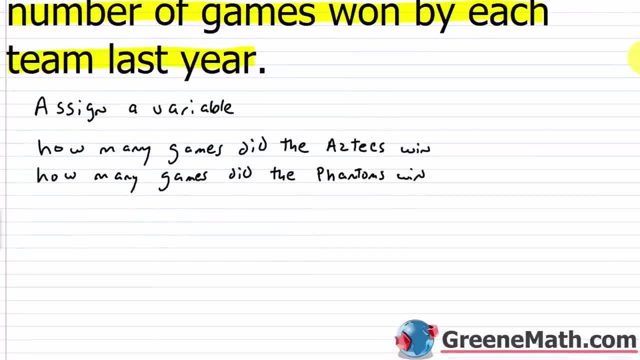 So when we get to this step, at this stage of assigning a variable, it really doesn't matter which one I assign a variable to. So in other words, we could say: let x equal the number of games the Aztecs won. Now you might be saying: 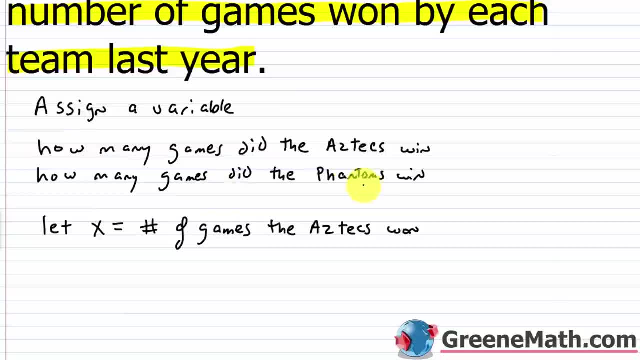 okay. well, if x equals the number of games that the Aztecs won, what are you going to do about the Phantoms? Well, you're going to express the number of games that the Phantoms won in terms of this variable x. 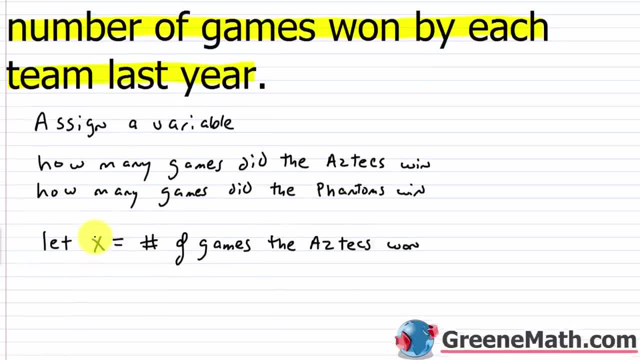 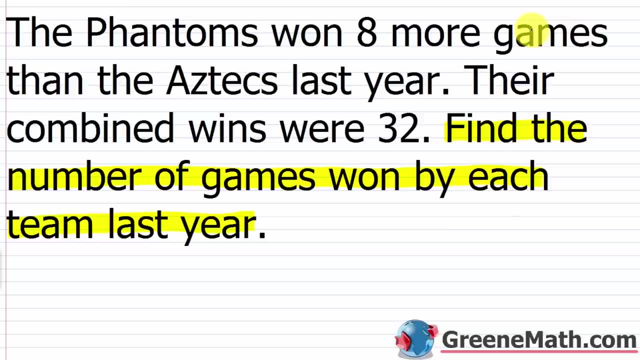 So let me show you how to do that. Let's scroll up to the top. So if I let x equal the number of games that the Aztecs won, well, the Phantoms won eight more games than the Aztecs last year. 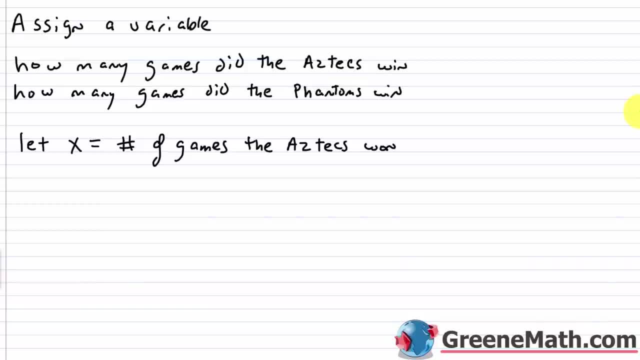 Again. let me kind of repeat this: x is the number of games the Aztecs won. The Phantoms won eight more than that. So I can just say that then x is the number of games the Aztecs won. 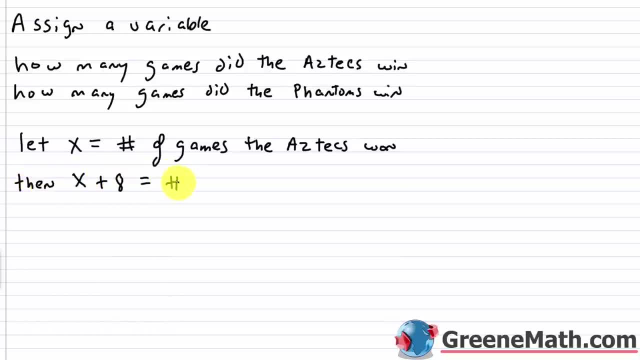 x plus eight is going to be equal to the number of games the Phantoms won. Very, very simple And I know at first it's a little confusing, but again, if you read back through the problem it makes perfect sense. 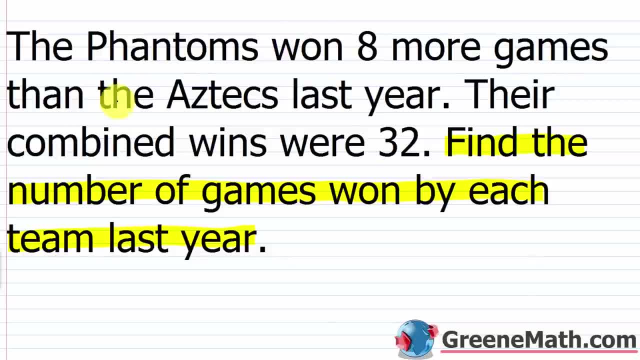 So let's go back up there. So the Phantoms won eight more games than the Aztecs last year. Okay, eight more. Their combined wins were 32.. Find the number of games the Aztecs won. The number of games won by each team last year. 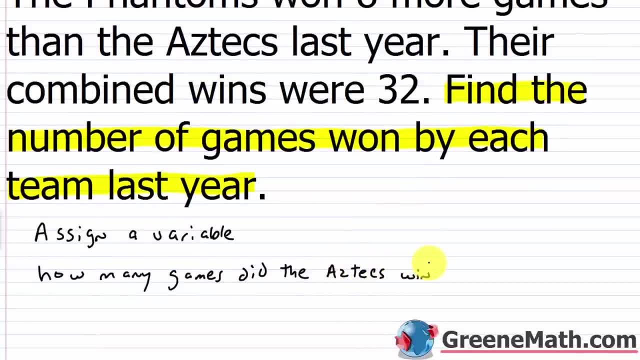 And then also how many games did the phantoms win? These are our two unknowns. 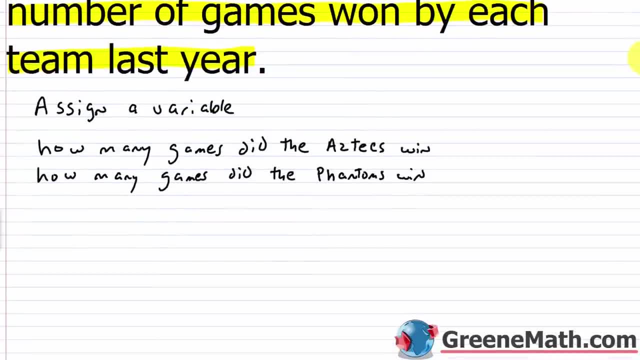 So when we get to the stage of assigning a variable, it really doesn't matter which one I assign a variable to. So in other words, we could say, let X equal the number of games. 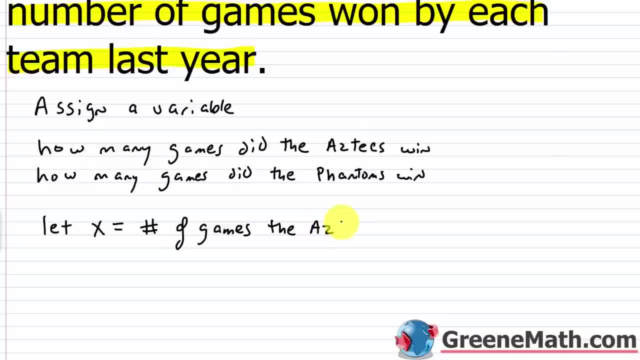 The Aztecs won. Now you might be saying, okay, 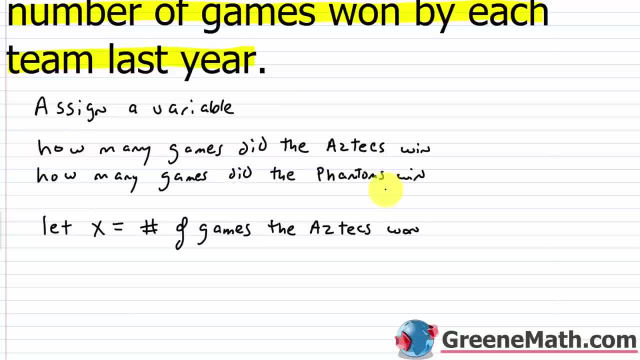 well if X equals the number of games that the Aztecs won, what are you going to do about the phantoms? Well, you're going to express the number of games that the phantoms won. In terms of this variable X. So let me show you how to do that. Let's scroll up to the top. 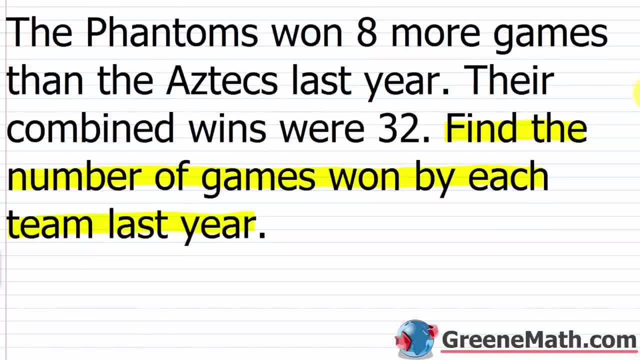 So if I let X equal the number of games that the Aztecs won, well, the phantoms won eight more games than the Aztecs last year. Again, let me kind of repeat this. X is the number of games the Aztecs won. The phantoms won eight more than that. 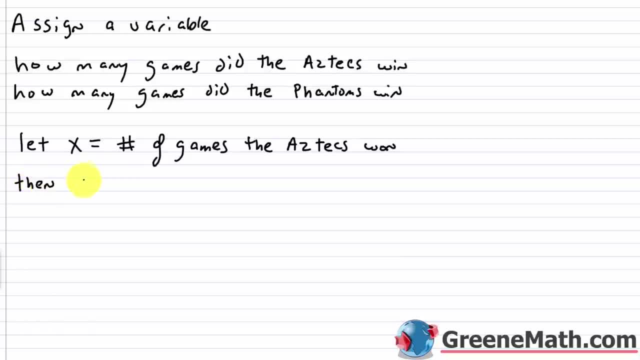 So I can just say that then X plus eight is going to be equal to the number. Of games. The phantoms won. Very, very simple. 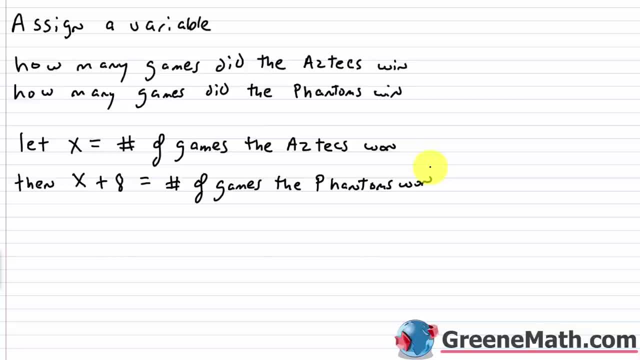 And I know at first it's a little confusing, but again, if you read back through the problem, it makes perfect sense. So let's go back up there. 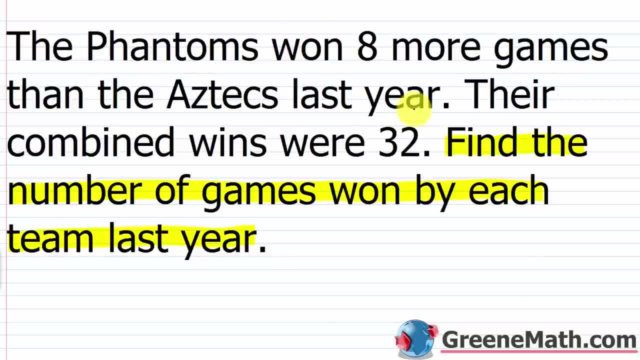 So the phantoms won eight more games than the Aztecs last year. Okay. Their combined wins were 32. Find the number of games won by each team last year. 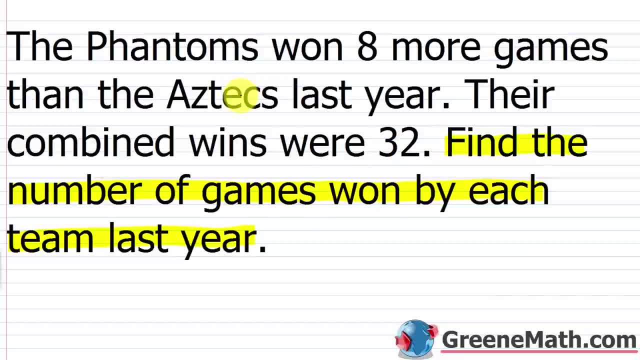 So again, if I'm letting X be the number of games that the Aztecs won last year, well, then X, that number again, 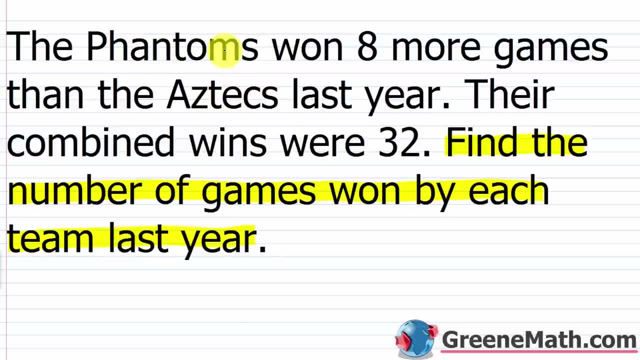 plus eight will be the number of games that the phantoms won. 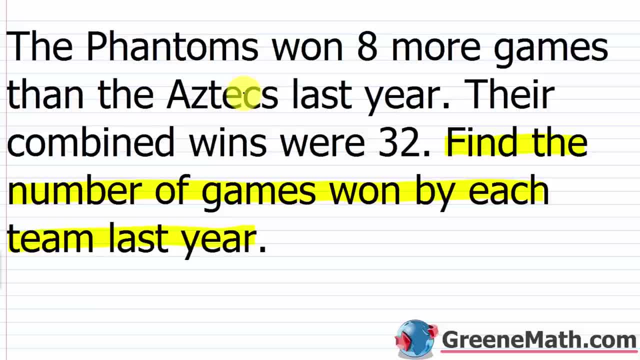 So again, if I'm letting x be the number of games that the Aztecs won last year, well then, x, that number again plus eight, will be the number of games that the Phantoms won. So now we have represented both of our unknowns. 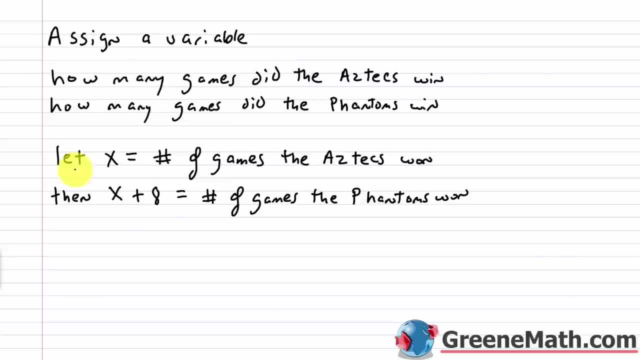 in terms of this one variable, x. okay. So again, we let x equal the number of games the Aztecs won, and so then, x plus eight is the number of games the Phantoms won. Now the next step is to write out. 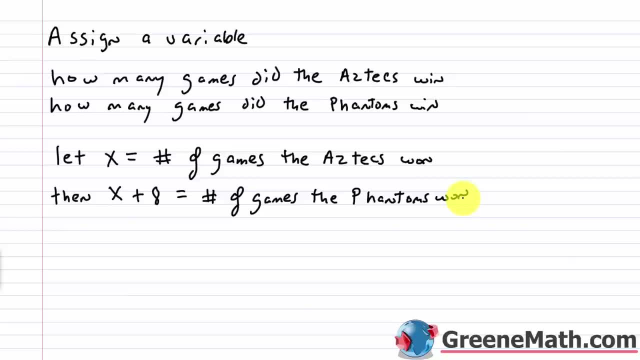 an equation, and in order to do that, you have to make use of the information given to you in the problem. So again, we're gonna read it one more time. So the Phantoms won eight more games than the Aztecs. 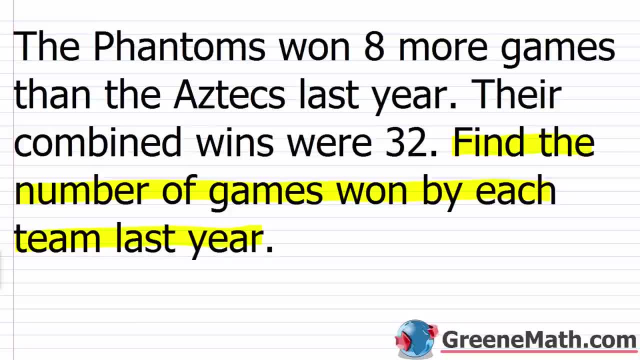 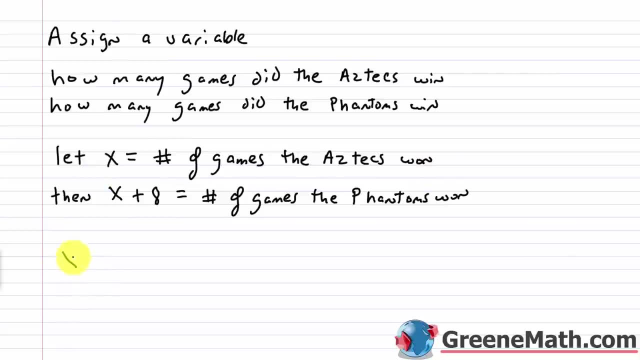 last year, Their combined wins- and this is key, right here- their combined wins were 32.. So if their combined wins were 32, that means that if I take the number of games that the Aztecs won, which is x, and I add to that, 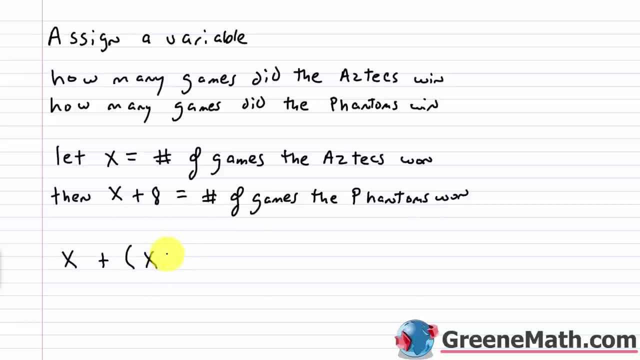 the number of games that the Phantoms won, which is x plus eight, that amount should be 32.. So that's how you go through and set up your equation. Again, this is the number of games that the Aztecs won. 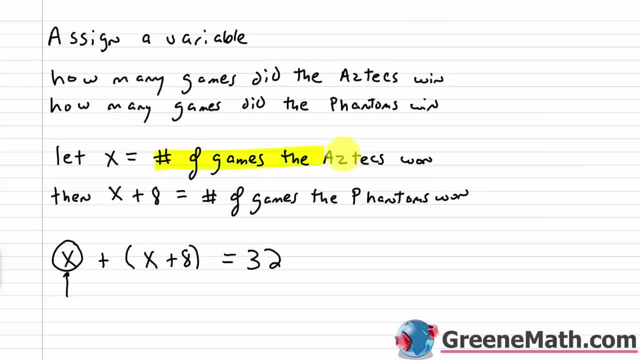 okay, number of games: number of games the Aztecs won. And then this is the number of games the Phantoms won. Number of games the Phantoms won. If I sum those two amounts together, their combined wins, I get 32,. right, this is the combined. 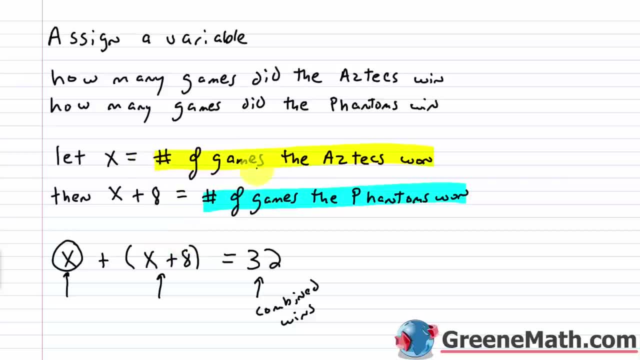 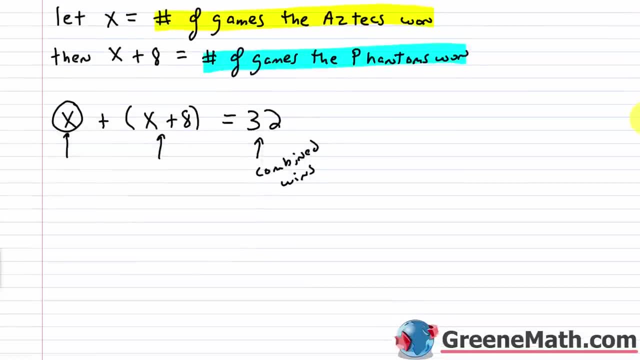 So I can go through and solve the equation. find the value of x, I'll know the number of games the Aztecs won. I can add eight to that value and find the number of games the Phantoms won. Let's go ahead and crank this out. 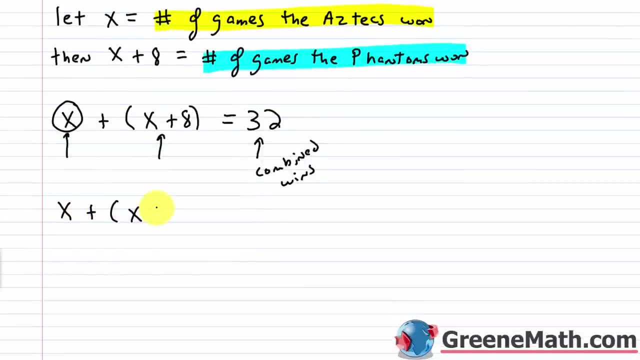 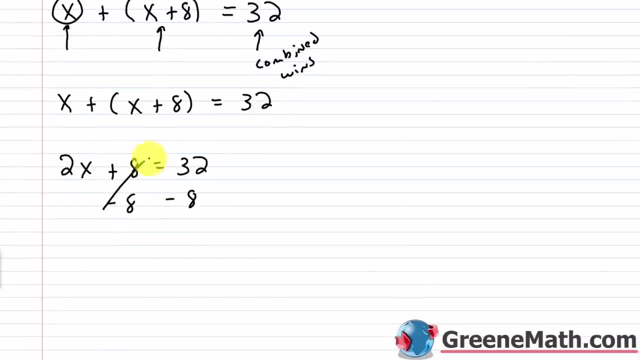 So if we have x plus this quantity, x plus eight, so we'd have x plus x, that's two x plus eight equals 32.. Subtract eight away from each side of the equation. This will cancel and we'll have two x equals. 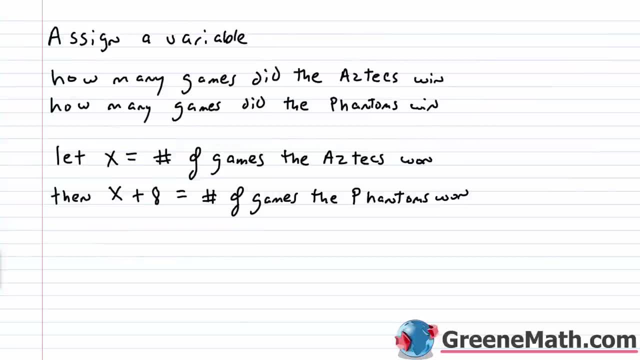 So now we have represented both of our unknowns in terms of this one variable X. Okay. So again, we let X equal the number of games the Aztecs won. 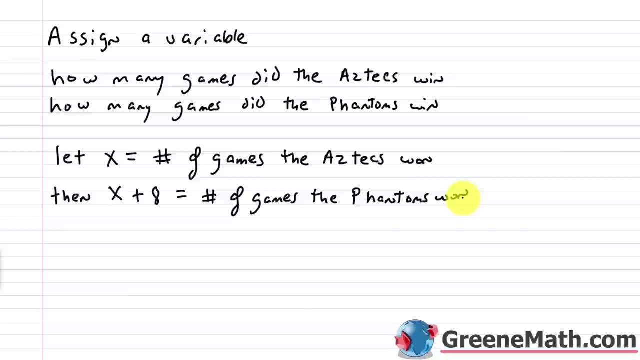 And so then X plus eight is the number of games the phantoms won. Now, the next step is to write out an equation. And in order to do that, 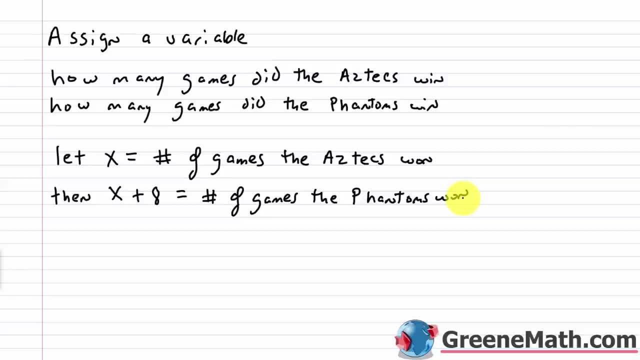 you have to make use of the information given to you in the problem. So again, we're going to read it one more time. 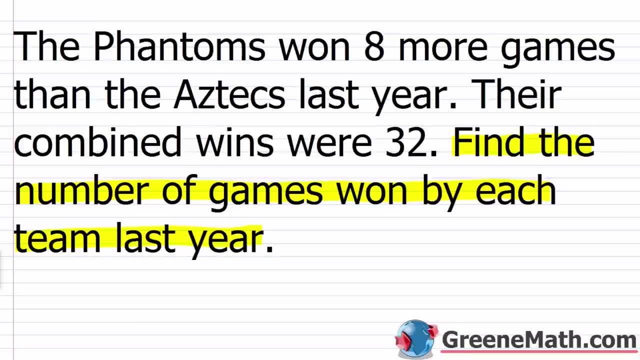 So the phantoms won eight more games than the Aztecs last year. Their combined wins, and this is key right here, their combined wins were 32. 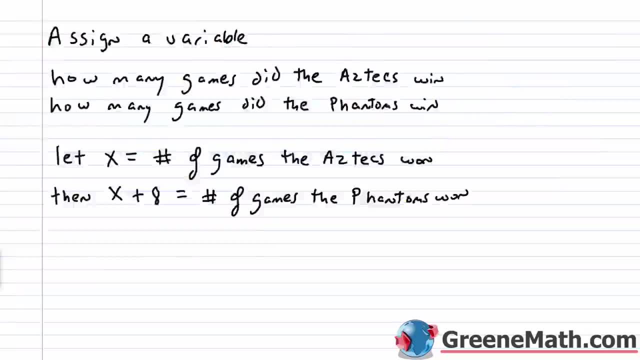 So if their combined wins were 32, that means that if I take the number of games that the Aztecs won, which is X, and I add to that, the number of games that the phantoms won, which is X plus eight, that amount should be 32. 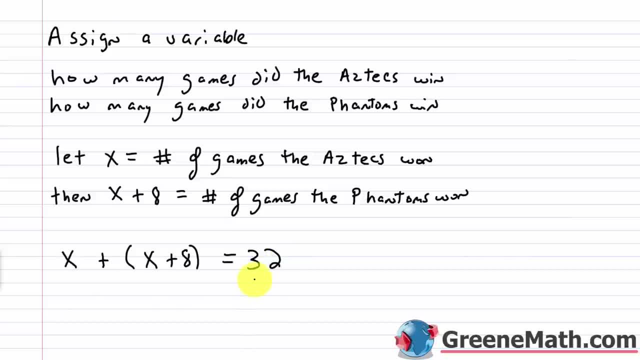 So that's how you go through and set up your equation. Again, this is the number of games that the Aztecs won. Okay. 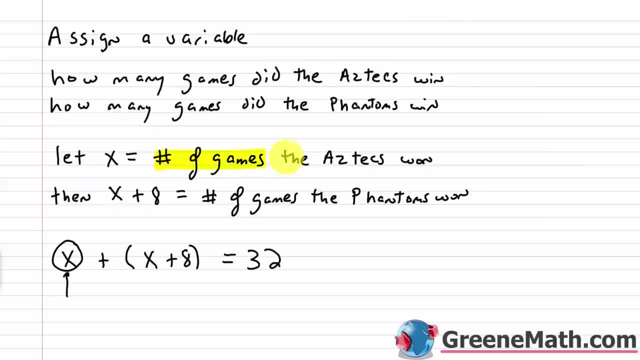 Number of games, number of games the Aztecs won. And then this is the number of games the phantoms won. 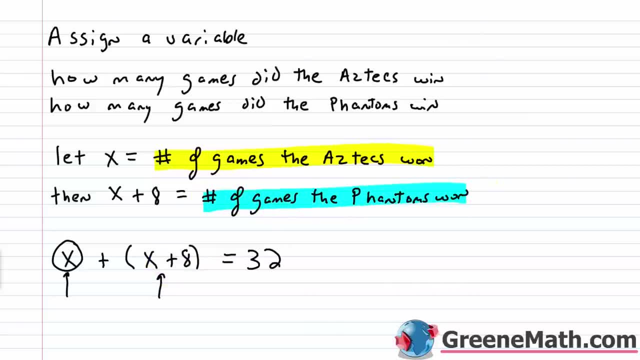 Number of games the phantoms won. If I sum those two amounts together, their combined wins, their combined wins, I get 32. 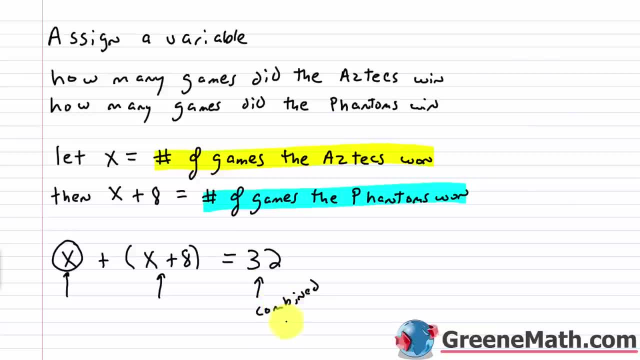 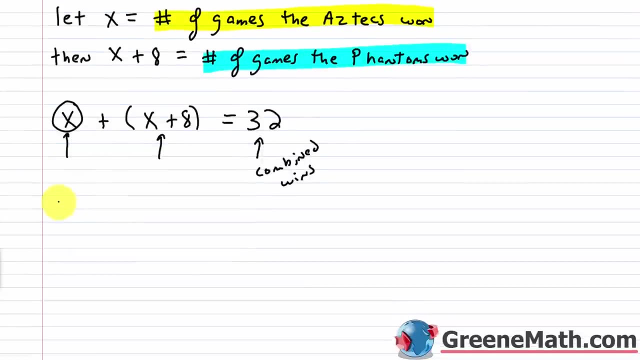 This is the combined. So I can go through and solve the equation, find the value of X. I'll know the number of games the Aztecs won. I can add eight to that value and find the number of games the phantoms won. Let's go ahead and crank this out. So if we have X plus this quantity, X plus eight, so we'd have X plus X, that's two X, plus eight equals 32. 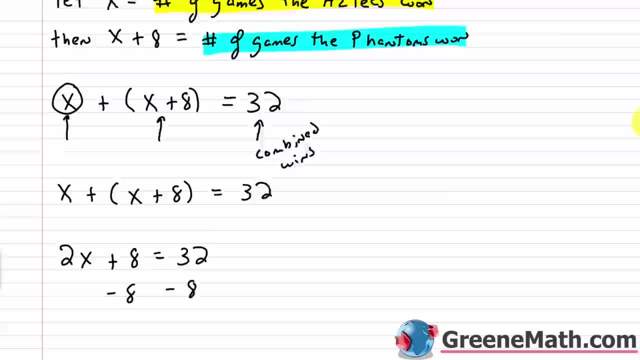 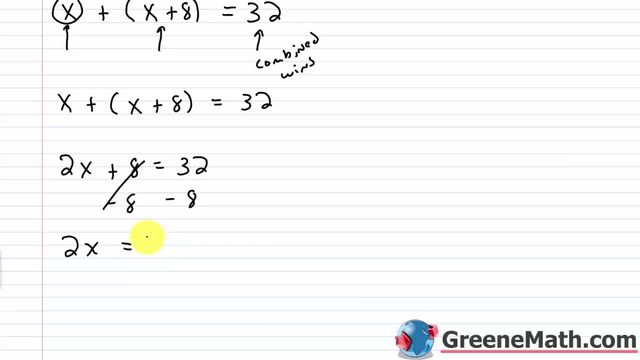 Subtract eight away from each side of the equation. This will cancel. And we'll have two X equals 32 minus eight is 24. 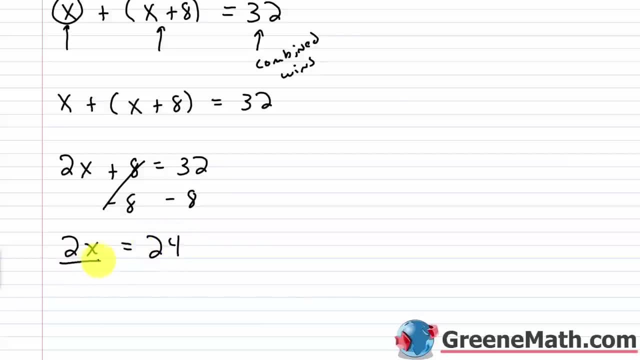 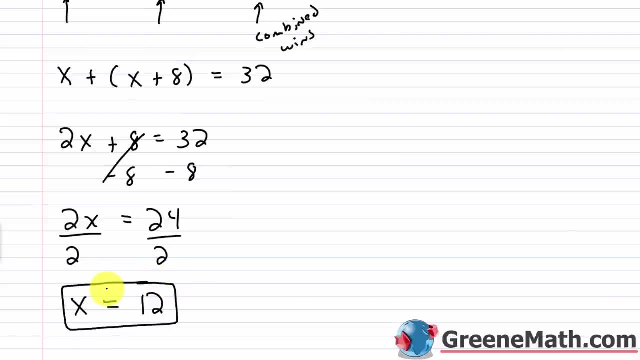 32 minus eight is 24.. Divide both sides of the equation by two and I'll have: x is equal to 12.. So again, what does that mean? X equals 12 is not the solution. Don't circle that on your paper and go, I'm done. 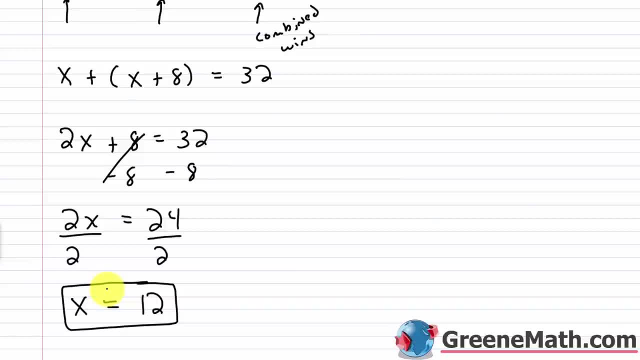 You're not, because with a word problem you have additional work. You have to go through and make sense of your answer. So that's why, after we finish step number four, solving the equation for step five, you're gonna state the answer. 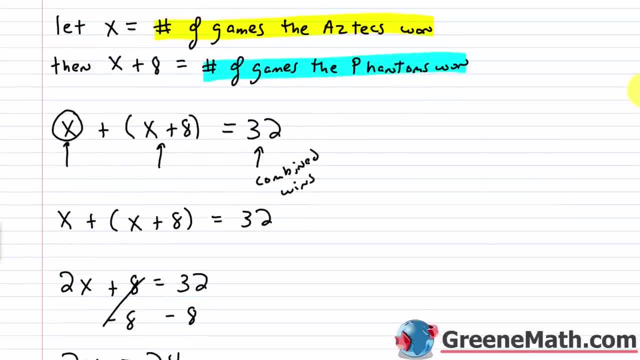 And in order to be able to state the answer, you've gotta be able to go back up and make sense of it. So x is the number of games the Aztecs won. So that means the Aztecs won 12 games. 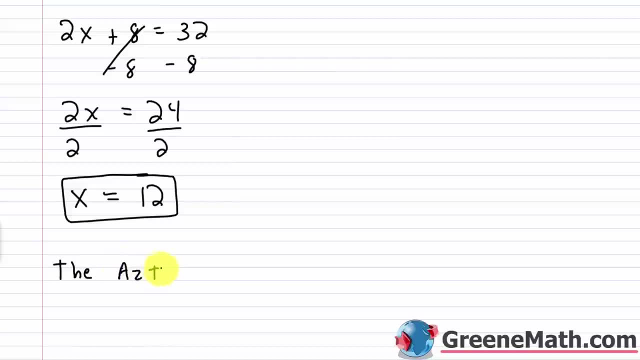 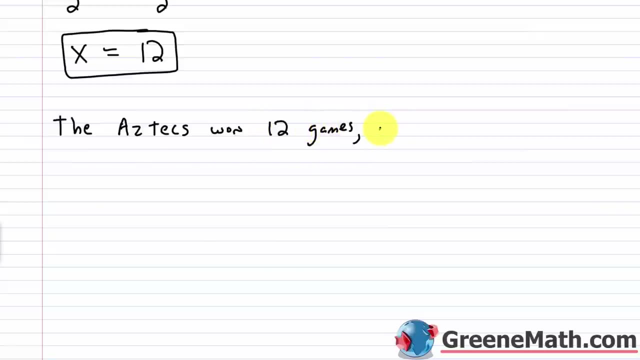 So the Aztecs won 12 games, While the Phantoms won. remember they won eight more games. So 12 plus eight is 20, right? Remember you had x plus eight to represent the number of games that the Phantoms won. 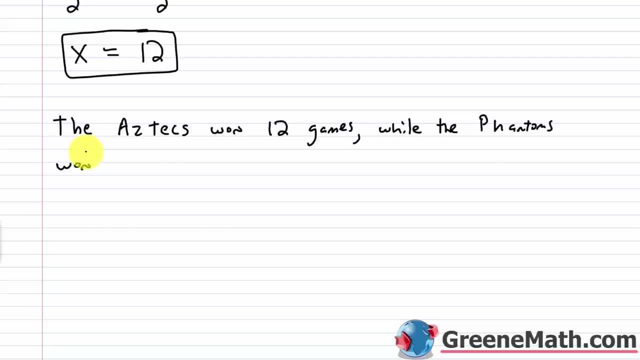 12 is x. So we now know the value for x, which is 12.. Plug that in 12 plus eight would be 20.. So while the Phantoms won 20 games, 12 plus eight is 20.. 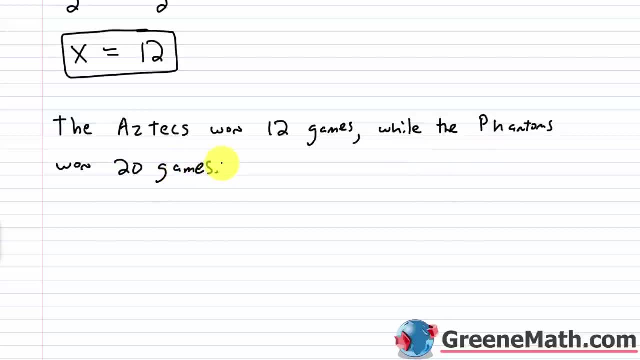 So the Aztecs won 12 games, while the Phantoms won 20 games. So now you've answered your word problem And you just wanna read back through the problem and make sure that your answer makes sense. So the Phantoms won eight more games. 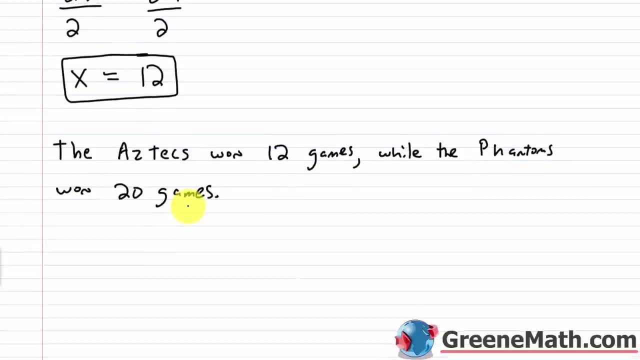 than the Aztecs last year. Well yeah, the Phantoms won 20 games, The Aztecs won 12.. 12 plus eight is 20.. So that checks out. Their combined wins were 32.. 12 plus 20 is 32.. 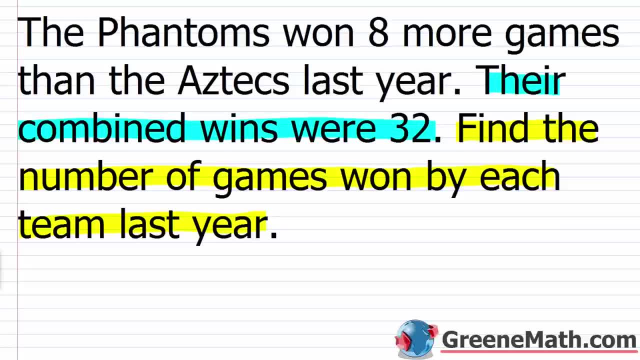 So that checks out also. So it looks like we have the correct answer. So we're gonna go back to the original question. So the answer is the Phantoms won 20 games, while the Aztecs won 20 games. 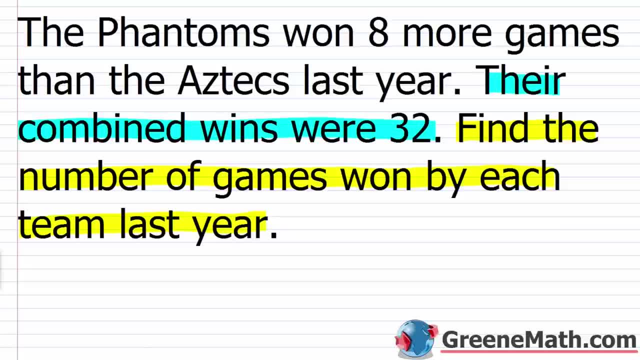 So the answer is: the Aztecs won 20 games, while the Phantoms won 20 games, So that checks out. Their combined wins were 32.. 12 plus 20 is 32.. So that checks out also. 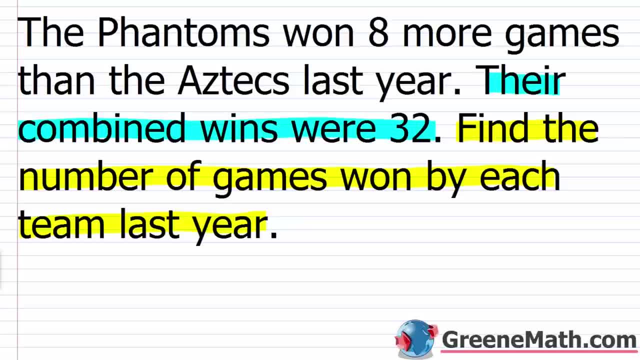 So it looks like we have the correct answer Again. the Phantoms won 20 games And the Aztecs won 12.. So one question you might have is: what if I started out by saying, okay, well, the number of games that the Phantoms won? 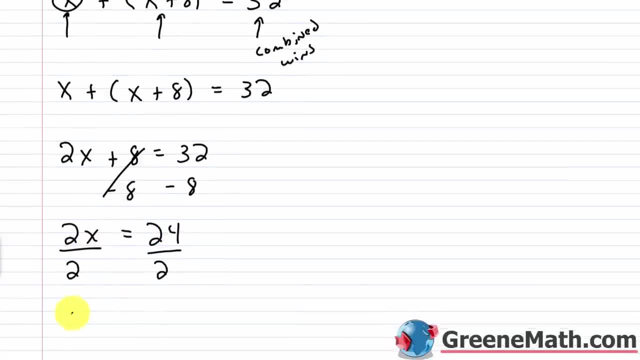 Divide both sides of the equation by two. And I'll have X is equal to 12. 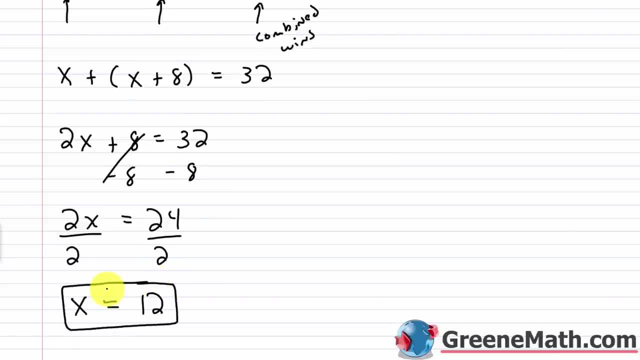 So again, what does that mean? X equals 12 is not the solution. Don't circle that on your paper and go, I'm done. You're not. 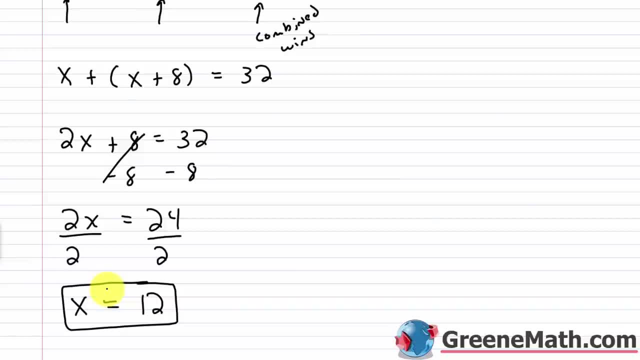 Because with a word problem, you have additional work. You have to go through and make sense of your answer. 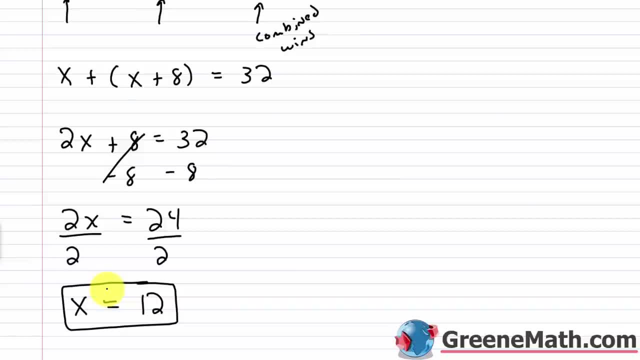 So that's why after we finish step number four, solving the equation, for step five, you're going to state the answer. And in order to be able to state the answer, you've got to be able to go back up and make sense of it. 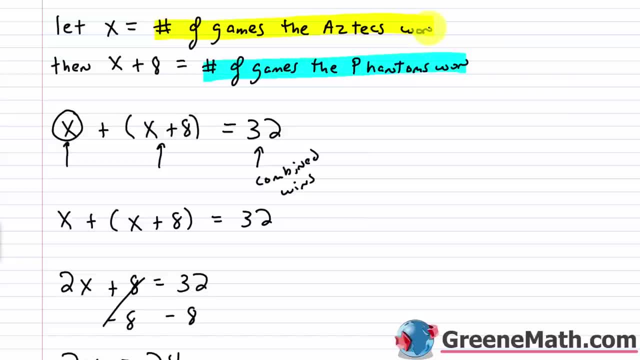 So X is the number of games the Aztecs won. So that means the Aztecs won 12 games. 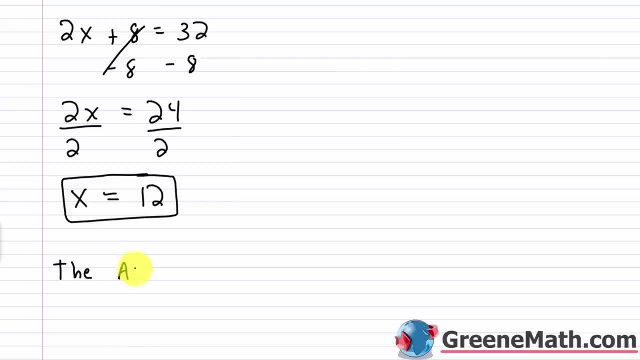 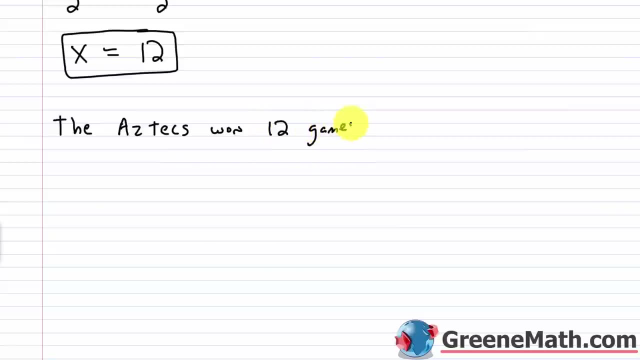 So the Aztecs, won 12 games. 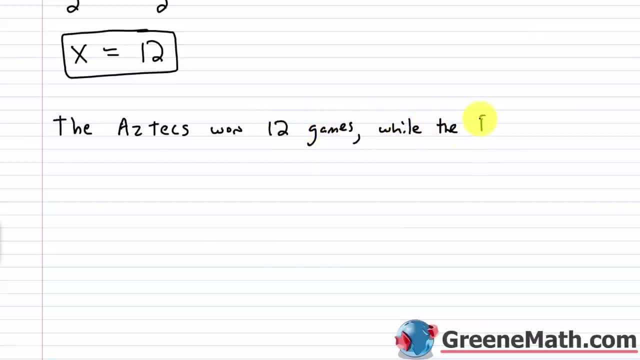 While the Phantoms won, remember they won eight more games. 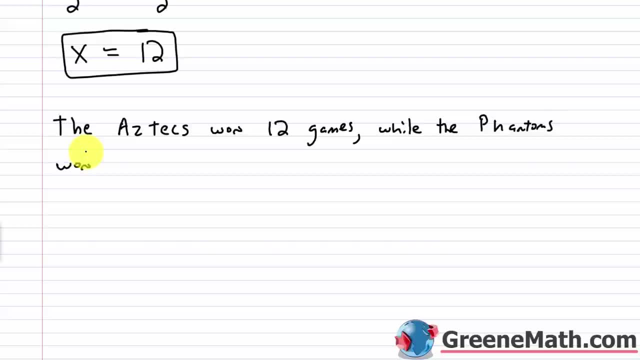 So 12 plus eight is 20, right? Remember you had X plus eight to represent the number of games that the Phantoms won. 12 is X. So we now know the value for X, which is 12. Plug that in. 12 plus eight would be 20. 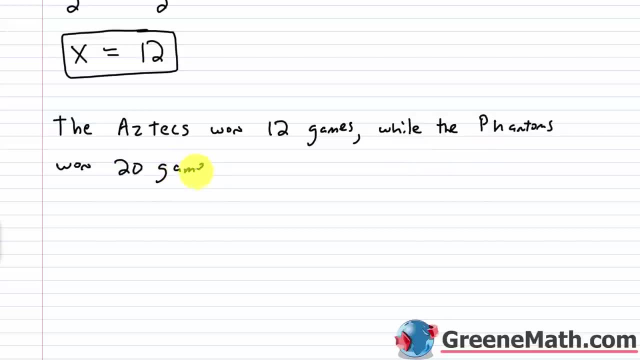 So while the Phantoms won 20 games. 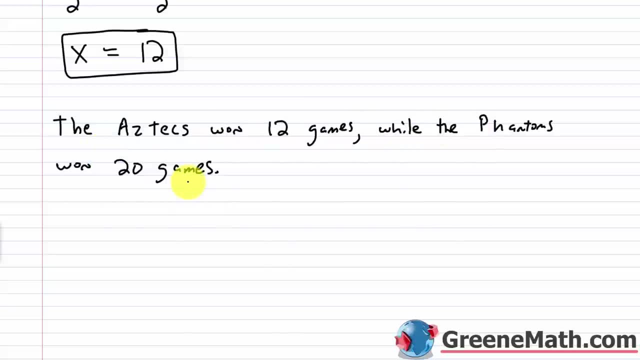 So the Aztecs won 12 games while the Phantoms won 20 games. 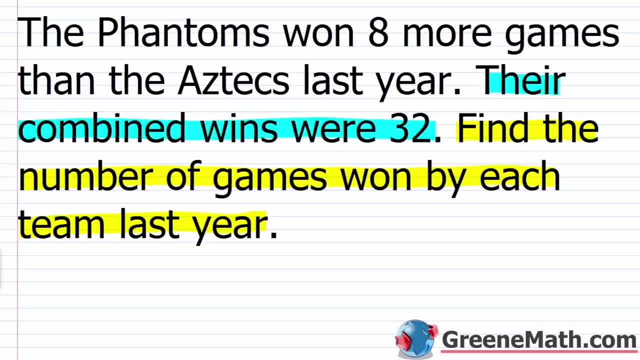 So now you've answered your word problem. And you just want to read back through the problem and make sure that your answer makes sense. So the Phantoms won eight more games than the Aztecs last year. 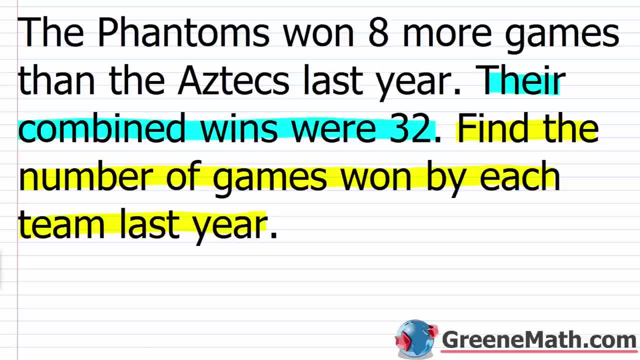 Well, yeah, the Phantoms won 20 games. The Aztecs won 12. 12 plus eight is 20. So that checks out. Their combined wins were 32. 12 plus 20 is 32. So that checks out also. So it looks like we have the correct answer. 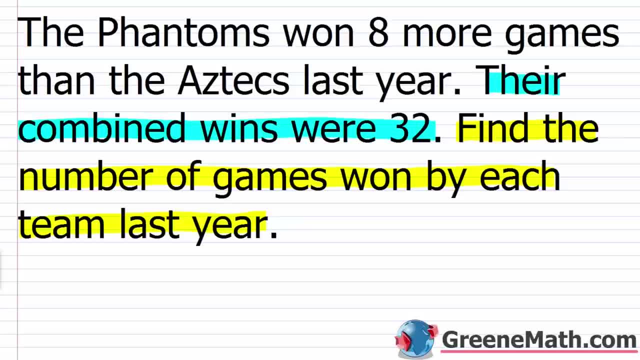 Again, the Phantoms won 20 games and the Aztecs won 12. So one question you might have is what if I started out by saying, okay, well, the number of games that the Phantoms won would be represented with X. So let's try it that way. 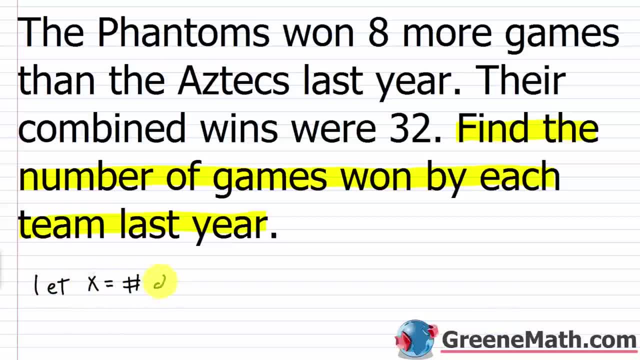 Let X equal the number of games the Phantoms won. So then X minus eight is now the number of games the Aztecs won. 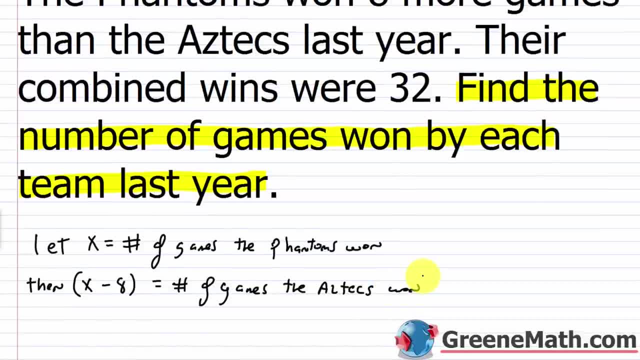 So you can do it either way. It doesn't really matter. You're going to get the same answer. 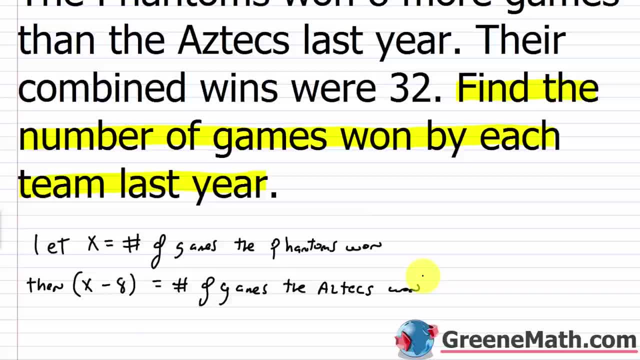 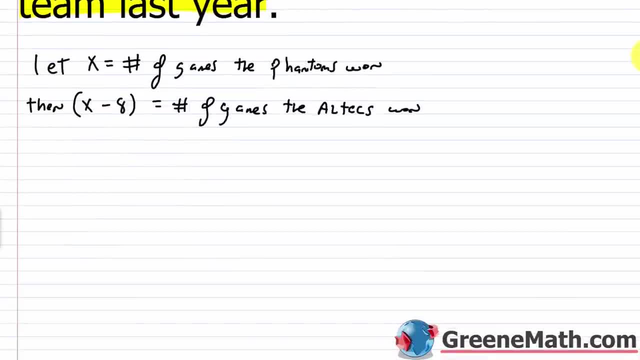 So we let X equal the number of games the Phantoms won. And so then X minus eight is the number of games the Aztecs won. And again, their combined wins were 32. So I can do the same thing as far as setting up an equation. So X plus this quantity X minus eight equals 32. X plus X is 2X minus eight equals 32. Add eight to both sides of the equation. That's gone. I'll have 2X is equal to 40. 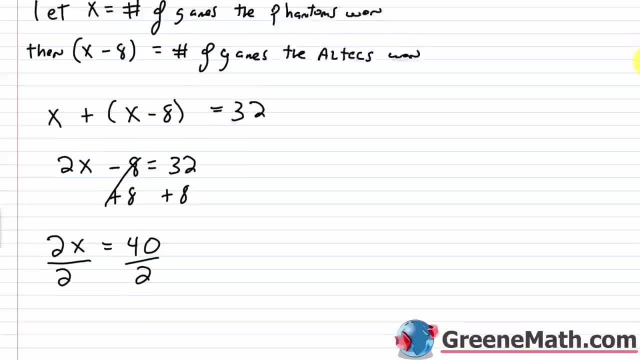 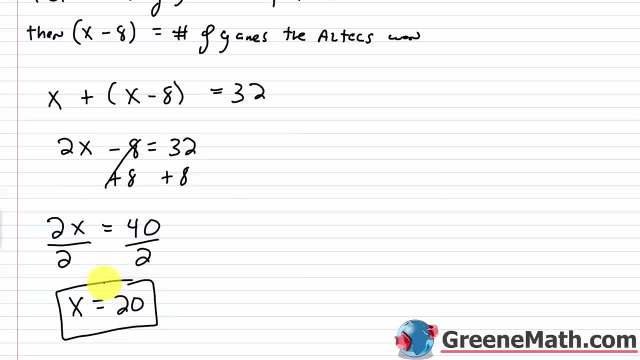 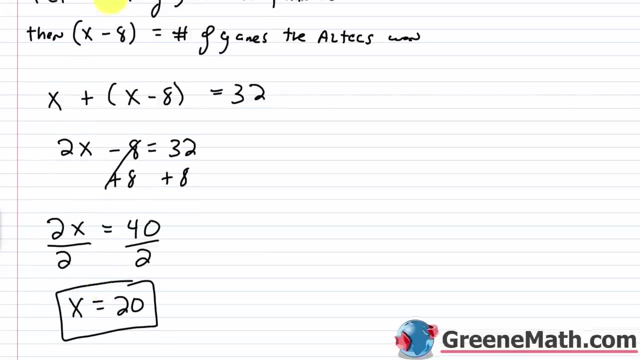 Divide both sides of the equation by two. And what I'm going to have now is that X equals 20. And you might say, well, you got a different answer. Before you said X equals 12. Remember, we changed what X was representing. So, of course, the answer is going to change. But we still got the correct answer and the same answer as before. X equals 20 here because, again, we let X equal the number of games the Phantoms won. Okay. 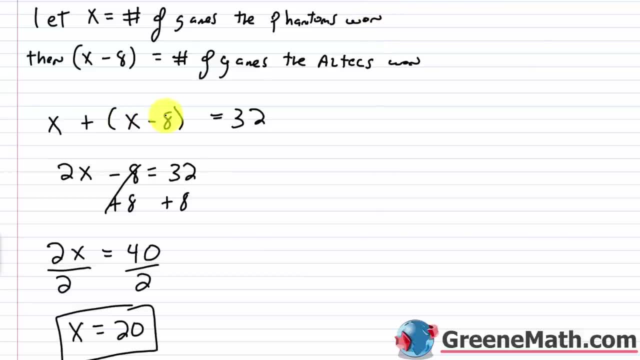 So the Phantoms won 20 games. And then X minus eight is the number of games the Aztecs won. So 20 minus eight is 12. So, again, you get the same answer. 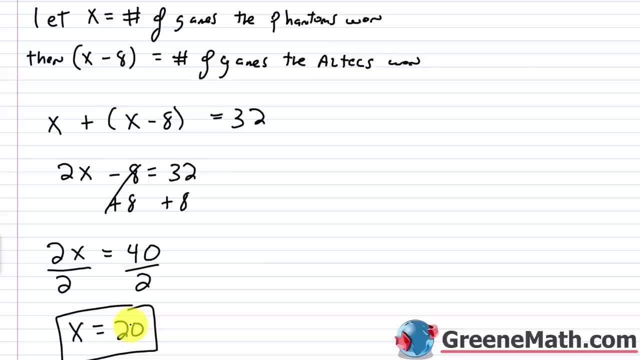 The Phantoms won 20 games. And the Aztecs won 20 minus eight or 20. They won 12 games. All right. Let's take a look at another one. 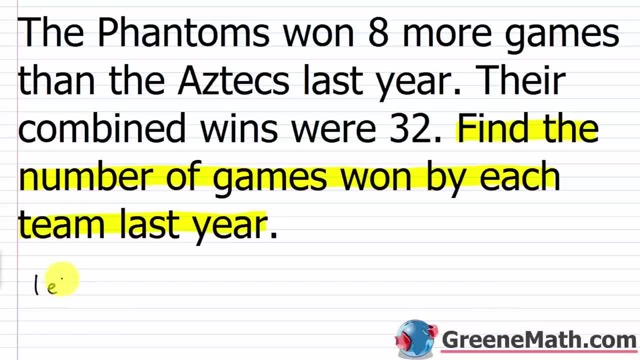 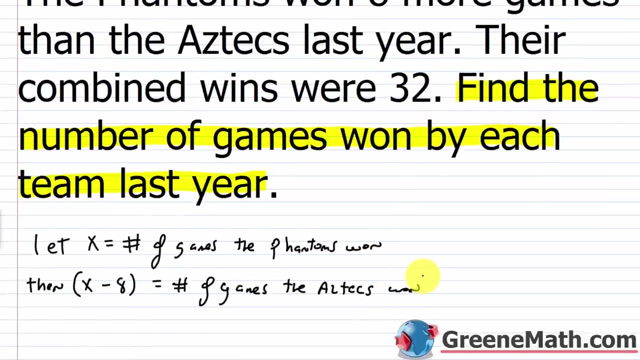 would be represented with X. So let's try it that way. Let X equal the number of games. I have the phantoms one. so then x minus eight is now the number of games, the aztecs one. so you can do it either way, it doesn't really matter, you're going to get the same answer. so 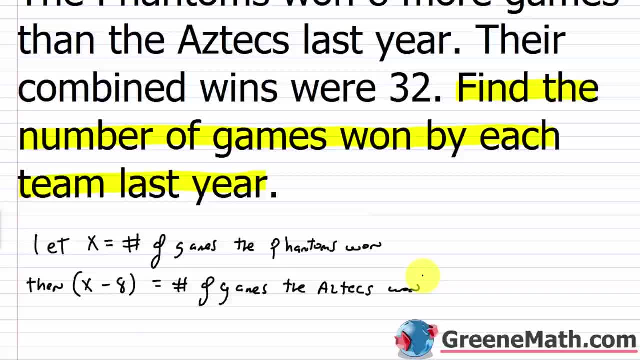 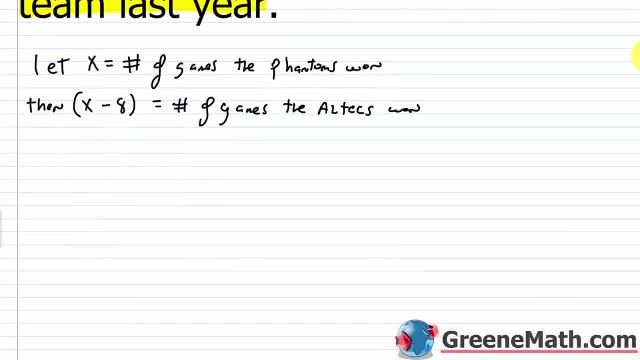 we let x equal the number of games, the phantoms one, and so then x minus eight is the number of games. the aztecs one and again, their combined wins were 32. so i can do the same thing as far as setting up an equation. so x plus this quantity, x minus eight, equals 32. x plus x is 2x minus 8. 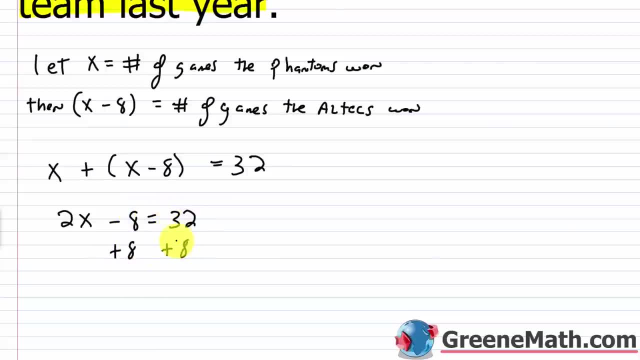 equals 32. add 8 to both sides of the equation. that's gone. i'll have: 2x is equal to 40. divide both sides of the equation by 2, and what i'm going to have now is that x equals 20, and you might say: well, you got a different. 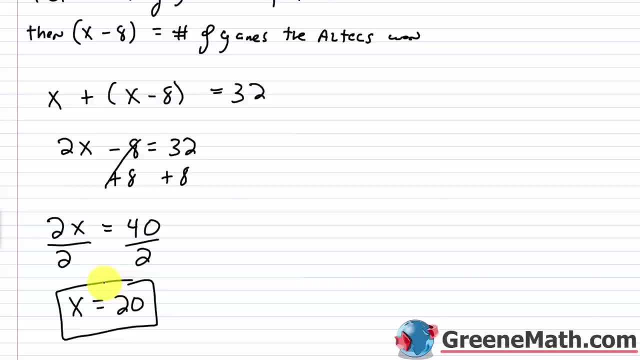 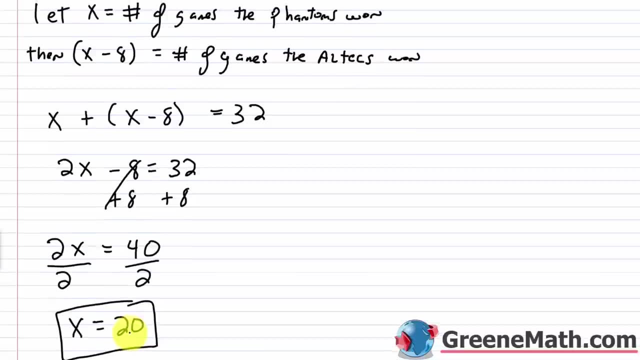 answer. before you said x equals 12. remember, we changed what x was representing, so of course the answer is going to change, but we still got the correct answer and the same answer as before. x equals 20. here because again, we let x equal the number of games the phantoms won. okay, so the 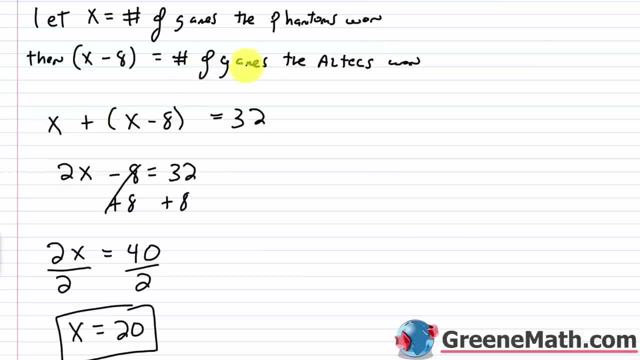 phantoms won 20 games, and then x minus 8 is the number of games the aztecs won. so 20 minus 8 is 12. so again you get the same answer as before and you might say: well, you got a different answer before. you said x. 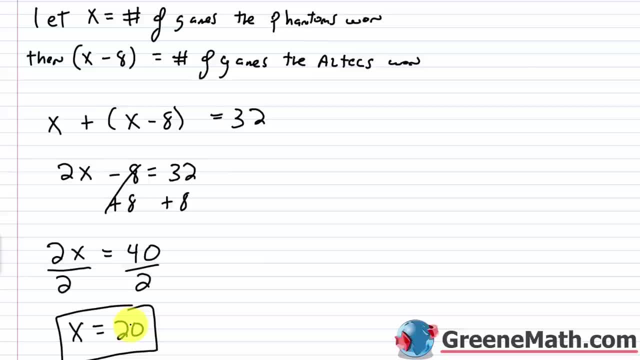 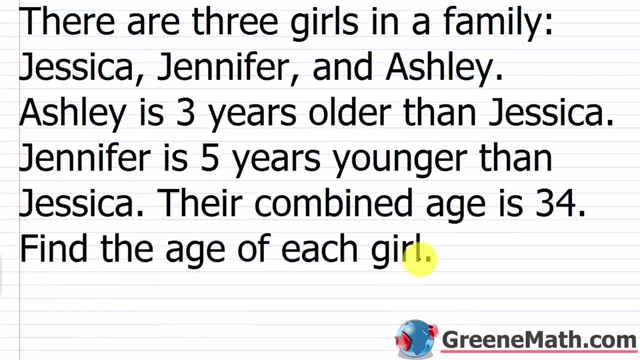 equals 20 and you got the same answer. the phantoms won 20 games and the aztecs won 20 minus 8 or 12 games. all right, let's take a look at another one. so there are three girls in a family we have. 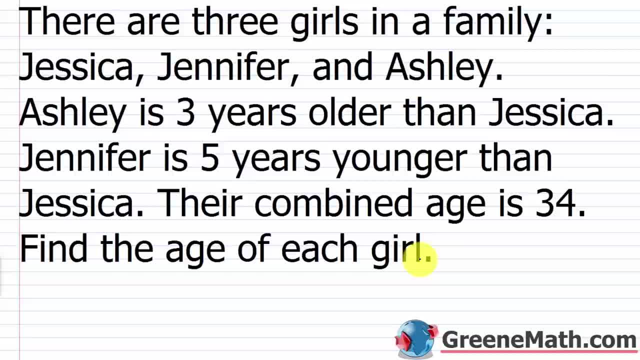 jessica, jennifer and ashley. ashley is three years older than jessica. jennifer is five years younger than jessica. their combined age is 34. find the age of each girl. so when you read this problem for the first time, again, your goal is to figure out what's the age of each girl and what's the. 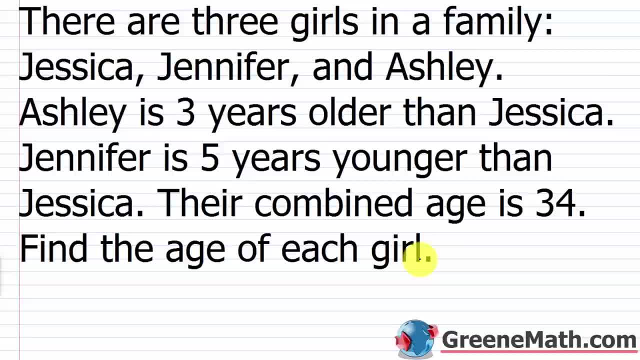 So there are three girls in a family. We have Jessica, Jennifer, and Ashley. Ashley is three years older than Jessica. Jennifer is five years younger than Jessica. Their combined age is 34. Find the age of each girl. 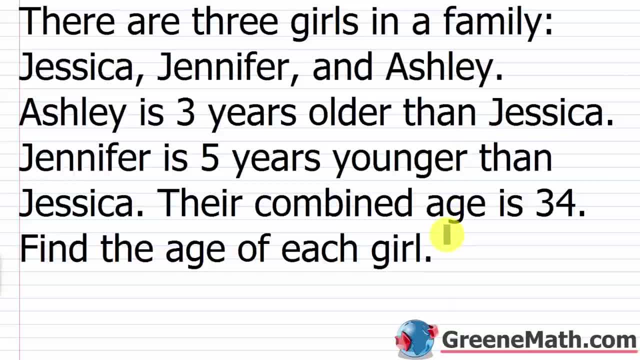 So when you read this problem for the first time, again, your goal is to figure out what you're being asked to find. We're being asked to find the age of each girl. This is another problem where we're trying to find the individual amounts given that we have the sum of the individual amounts. So their combined age is given to us. 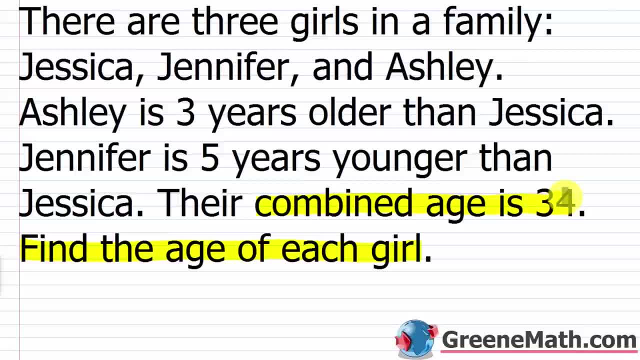 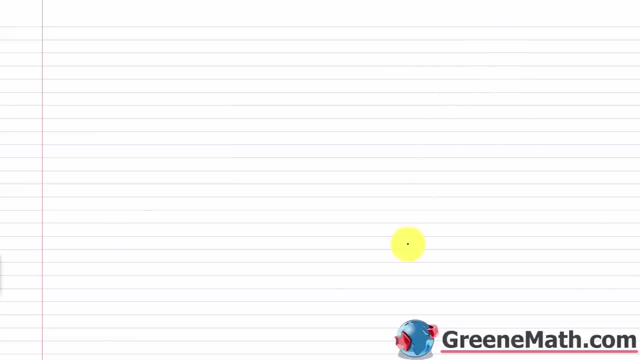 So if there are three girls, Jessica, Jennifer, and Ashley, they represent our three unknowns. We want to find the age of each one. So when we move on to our next step, which is to assign a variable to represent the unknown, well, you have three unknowns here. You don't know the age of Ashley. You don't know the age of Jessica. And you don't know the age of Jennifer. Now I'm going to set a variable equal to one of their ages. 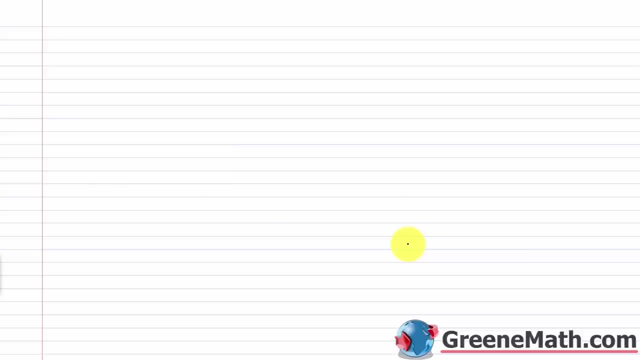 And then I'm going to express the other girls' ages in terms of that one variable. Now here's a little trick. 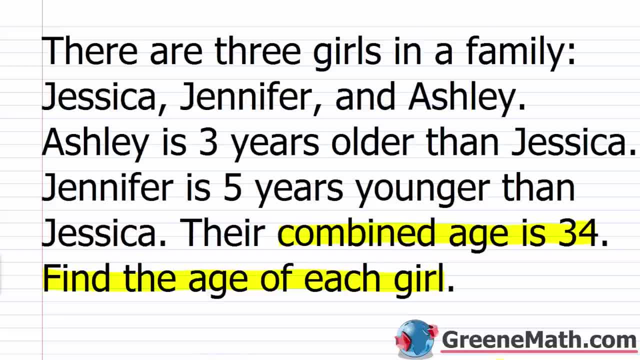 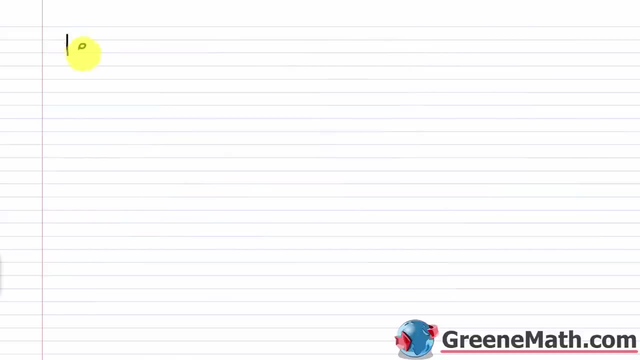 When you read through your problem, if you have one of the individuals that is involved in both comparisons. So in this case, you have Ashley is three years older than Jessica. And then Jennifer is five years younger than Jessica. So Jessica is three years older than Jessica. So Jessica is involved in the comparison with Ashley and also with Jennifer. So I'm going to go ahead and let x. I'm going to let x equal Jessica's age. 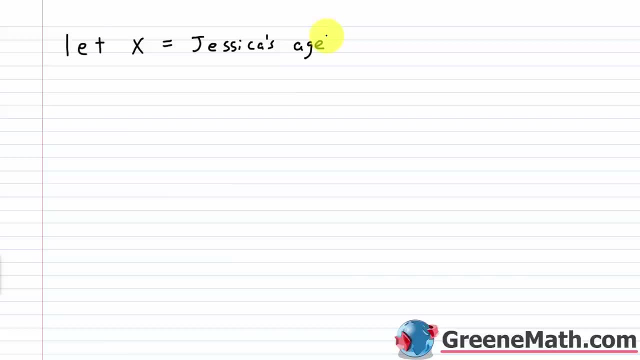 Now I can express the other girls' ages in terms of this variable x. So I can say then. If Ashley, we're told that Ashley is three years older than Jessica. 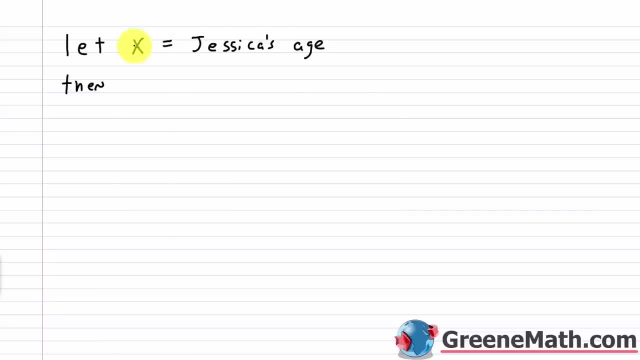 So if she's three years older than Jessica and Jessica's age is x. Well, then x, again, Jessica's age plus three is going to equal Ashley's age. 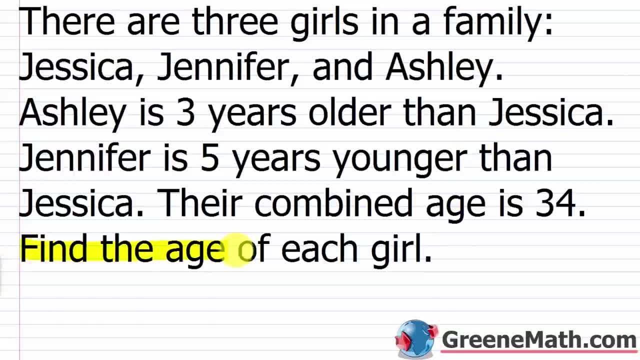 age of each girl we're being asked to find. we're being asked to find the age of each girl. this is another problem where we're trying to find the individual amounts, given that we have the sum of the individual amounts, so their combined age is given. to us it's 34, so if there are three girls, 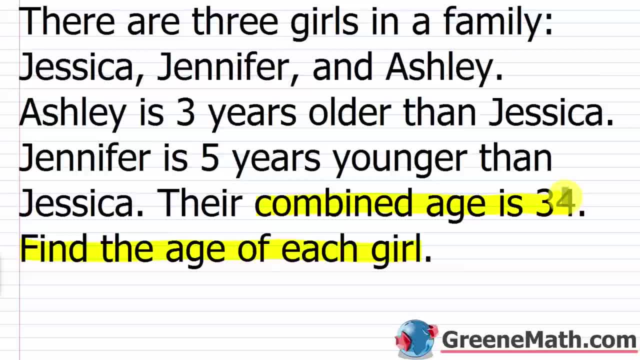 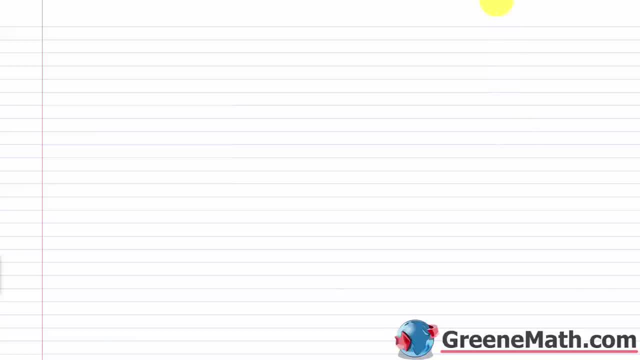 jessica, jennifer and ashley. they represent our three unknowns. we want to find the age of each one. so when we move on to our next step, which is to assign a variable to represent the age of each one, we're going to use the variable to represent the unknown. well, you have three unknowns here. 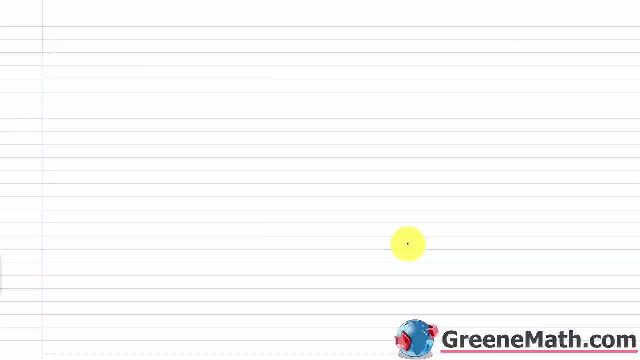 you don't know the age of ashley, you don't know the age of jessica and you don't know the age of jennifer. now i'm going to set a variable equal to one of their ages, and then i'm going to express the other girls ages in terms of that one variable. now here's a little trick when you read through: 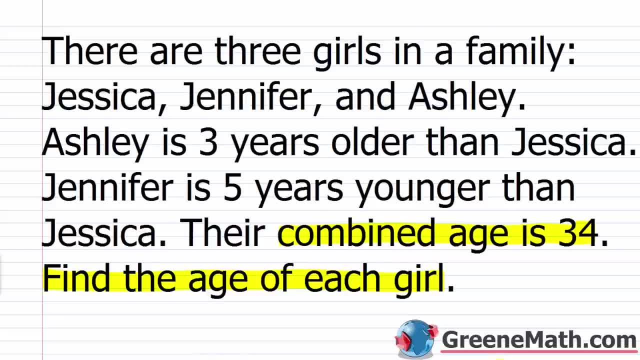 your problem if you have one of the individuals that is involved in both comparisons. so in this case you have: ashley is three years older than jessica and jessica is five years older than jessica, and then jennifer is five years younger than jessica, so jessica is involved in the comparison. 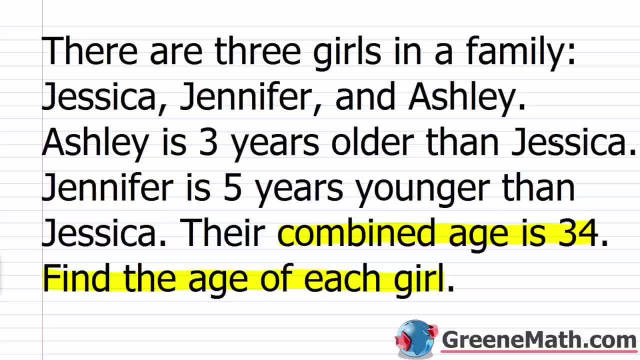 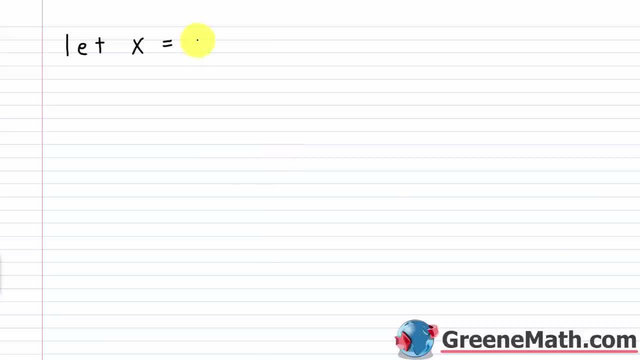 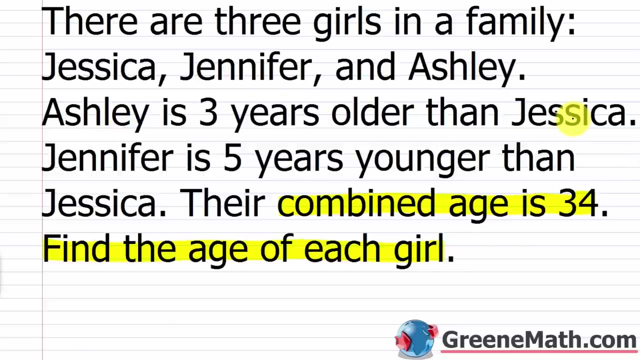 with ashley and also with jennifer. so i'm going to go ahead and let x. i'm going to let x equal jessica's age. now i can express the other girls ages in terms of this variable x. so i can say then, for ashley: we're told that ashley is three years older than jessica, so if she's three years older, 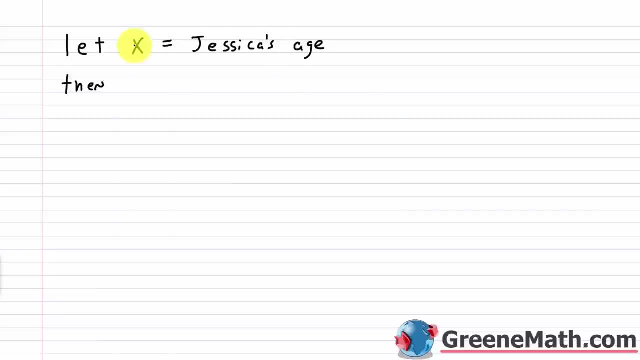 than jessica, and jessica's age is x. well then, x again. jessica's age plus three is going to equal ashley's age. and then what about jennifer? well, it's also telling me that jennifer is five years younger than jessica. 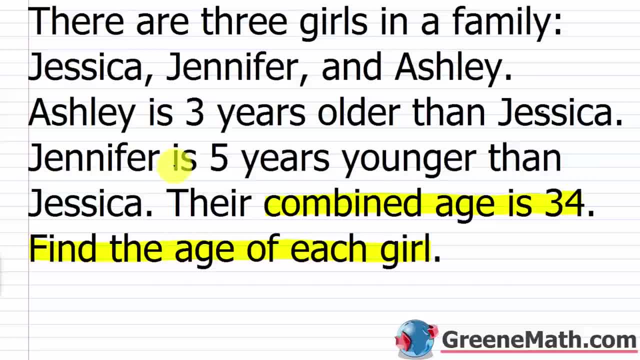 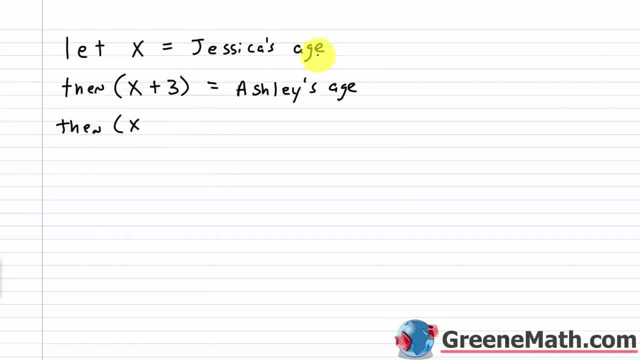 And then what about Jennifer? Well, it's also telling me that Jennifer is five years younger than Jessica. So that tells me. I can put then x, which again is Jessica's age, minus five. Minus five because Jennifer is five years younger. 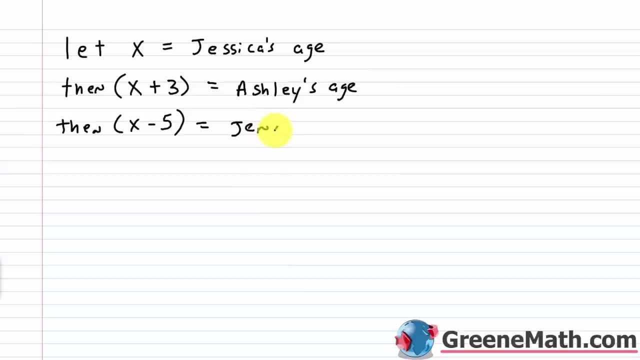 That's going to be Jennifer's age. So we have x as Jessica's age. Then we have x plus three as Ashley's age. Because Ashley is three years older than Jessica. And then we have x minus five as Jennifer's age. Again, because Jennifer is five years older than Jessica. Jennifer is five years younger than Jessica. All right. 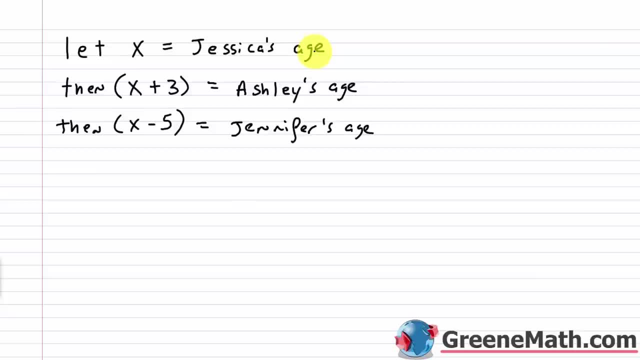 So in the next step, we're asked to set up an equation. So how do we set up an equation here? Well, again, just like we saw in the last problem. We have the sum of the individual amounts that are going to be equal to something. So if we look at the problem again, we're told that their combined age is 34. So what that means is if I take x, which is Jessica's age. And I add it to x plus three, which is Ashley's age. And then I add it to x minus five, which is Jennifer's age. I should get a value of 34. 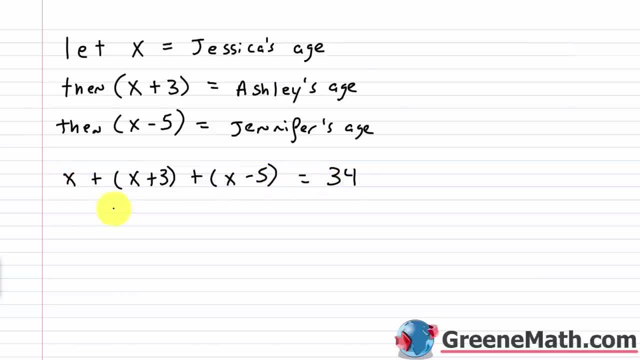 So we simplify this. x plus x plus x is three x. And then plus three minus five would be negative two. So I can put plus negative two. Or I can just put minus two. It doesn't really matter. So this is equal to 34. And then I'll add two to both sides of the equation. That's gone. And we'll have three x equals 34. 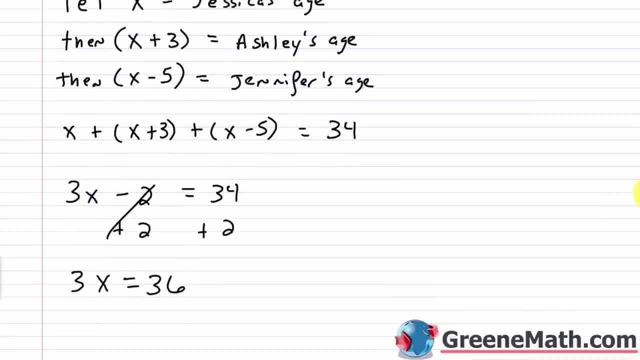 x equals 36. All right. 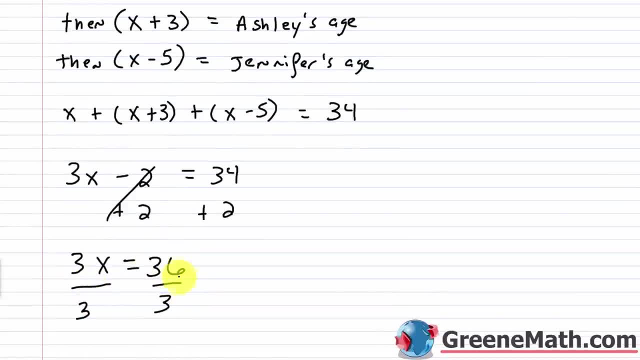 So now we'll divide both sides of the equation by three. So that x can be by itself. This will cancel with this. 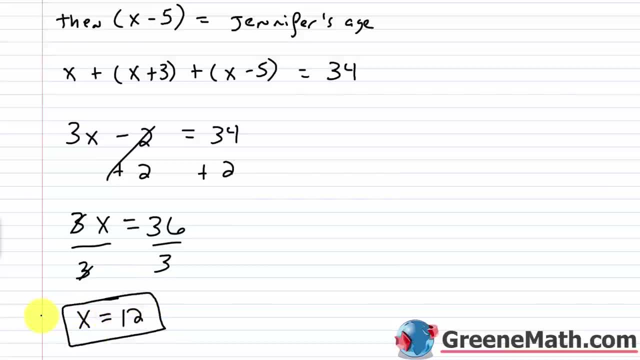 And I'll have x is equal to 12. 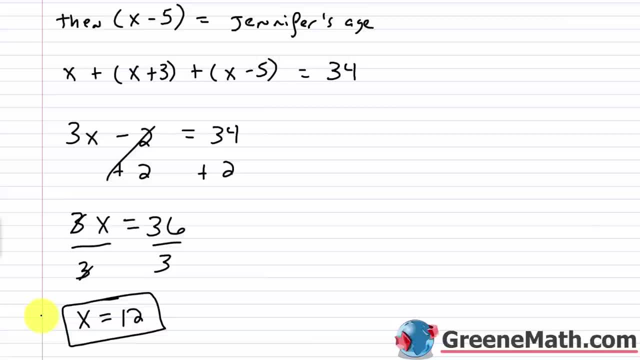 And you never thought that solving the equation would be the easy part. But now it's become that. 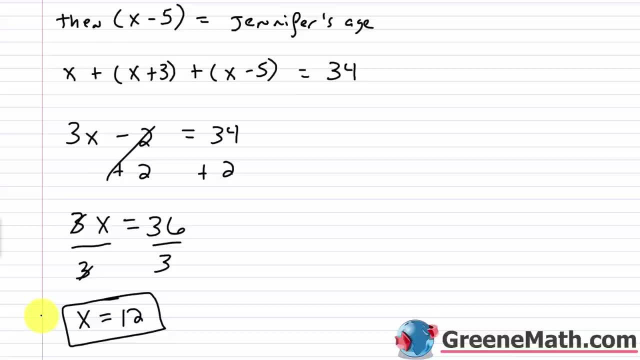 So I have x equals 12. But again, I'm not done. Please don't stop and turn your test in with this answer on. You will be wrong. 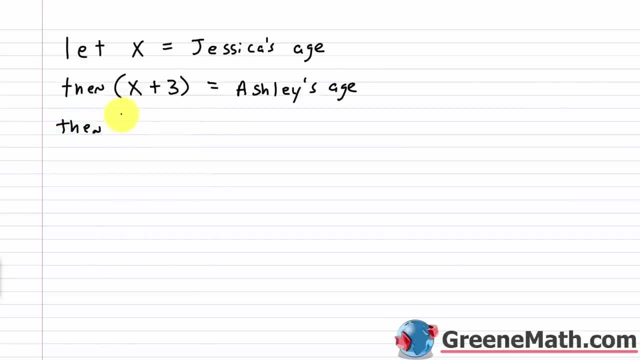 Jessica. So that tells me. I can put then x, which again is Jessica's age, minus 5, okay, minus 5, because Jennifer is five years younger. That's going to be Jennifer's age. So we have x as Jessica's age. Then we have x plus 3 as Ashley's age. right, because Ashley is. 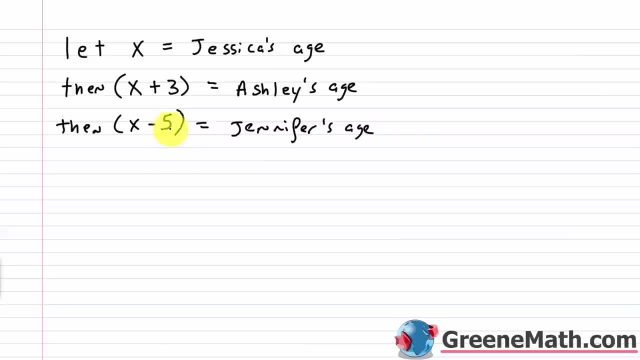 three years older than Jessica. And then we have x minus 5 as Jennifer's age again, because Jennifer is five years younger than Jessica. All right, so in the next step we're asked to set up an equation. So how do we set up an equation here? Well, again, just like we saw in the last problem, 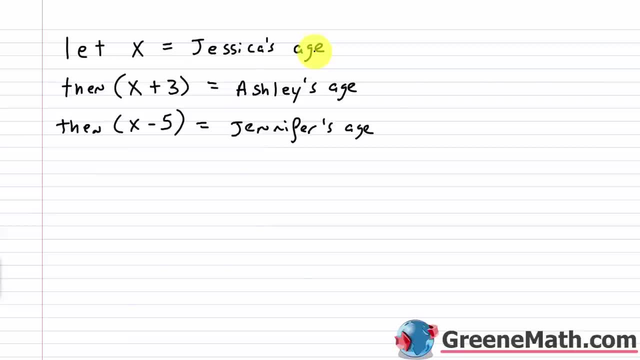 we have the sum of the individual amounts that are going to be equal to something. So if we look at the problem again, we're told that their combined age is 34.. So what that means is, if I take x, which is Jessica's age, and I take x minus 5,, which is Ashley's age, and I take x minus 5,. 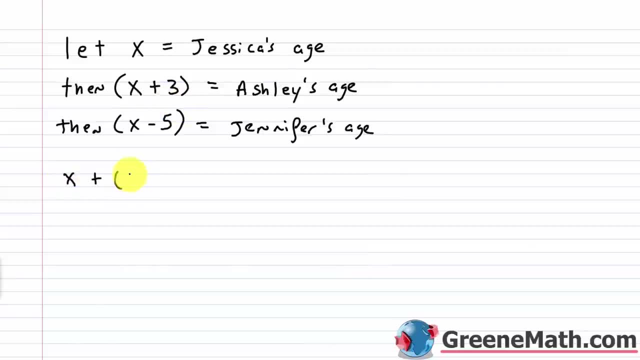 and I add it to x plus 3,, which is Ashley's age, and then I add it to x minus 5,, which is Jennifer's age, I should get a value of 34.. So we simplify this: x plus x. plus x is 3x, And then plus 3 minus. 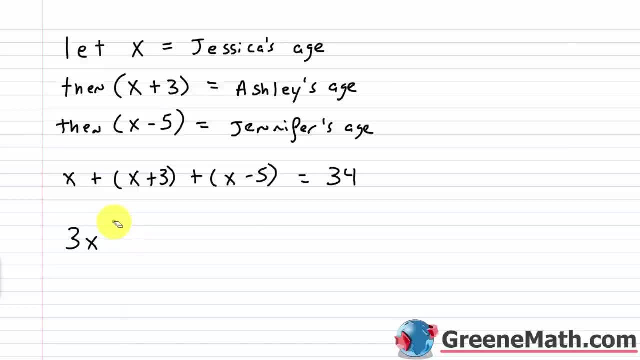 5 would be negative 2.. So I can put plus negative 2, or I can just put minus 2.. It doesn't really matter. So this is equal to 34.. And then I'll add 2 to both sides of the equation, And then I'll. 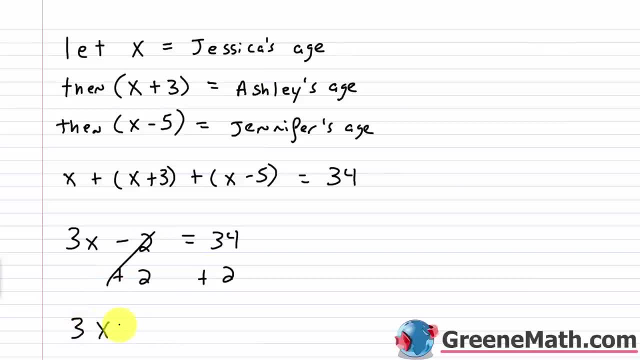 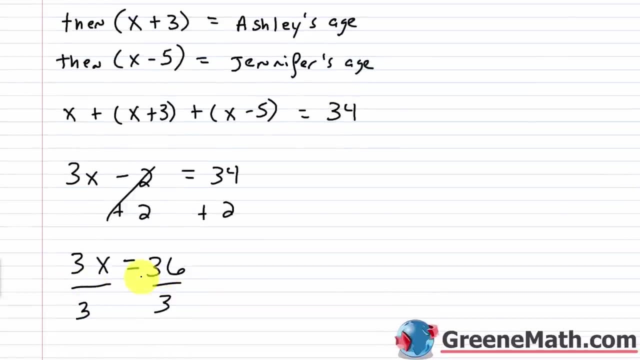 add 2 to both sides of the equation, That's gone And we'll have 3x equals 36.. All right, So now we'll divide both sides of the equation by 3 so that x can be by itself. This will cancel with. 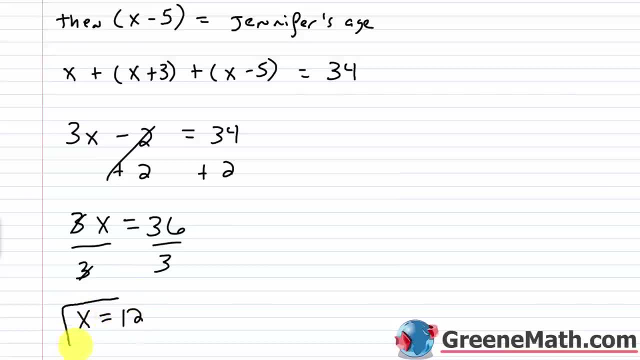 this And I'll have: x is equal to 12.. And you never thought that solving the equation would be the easy part, But now it's become that. So I have x equals 12.. But again, I'm not done. Please don't stop and turn your test in with this answer on. You will be wrong. 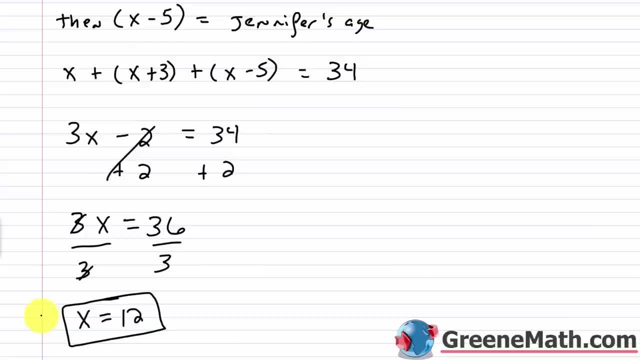 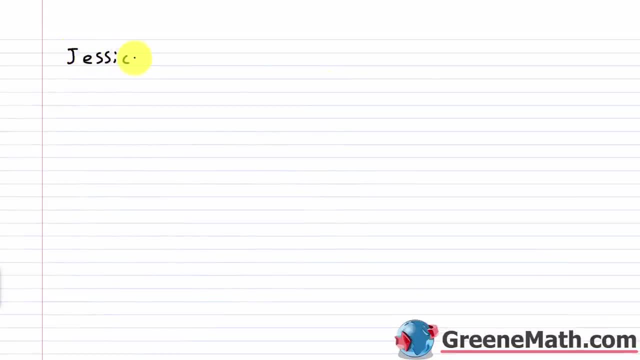 You have to translate this now into a sentence. So x equals 12.. x is Jessica's age. Jessica is 12 years old. Ashley, remember we represented her age with x plus 3, because she was 3 years older. Jessica is. 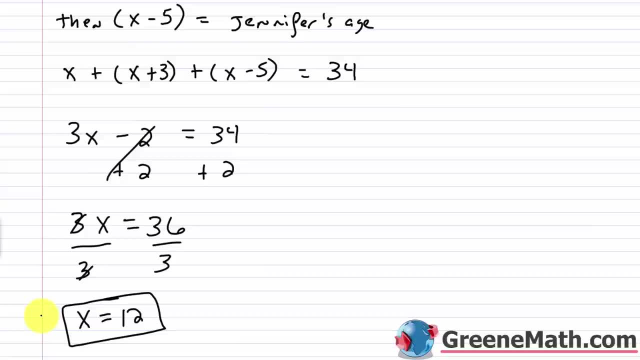 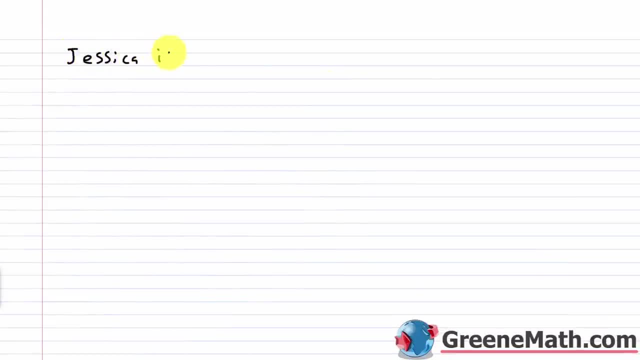 We have to translate this now into a sentence. So x equals 12. x is Jessica's age. Jessica is 12 years old. 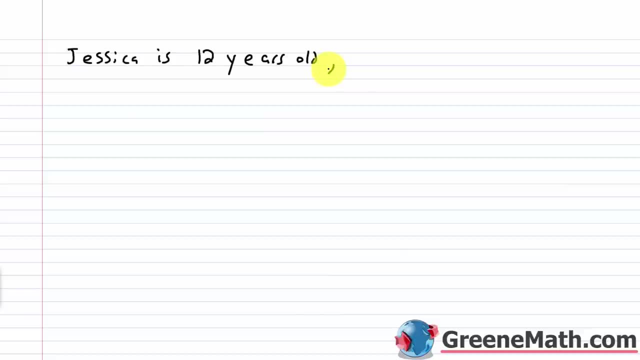 Ashley, remember, we represented her age with x plus three because she was three years older. 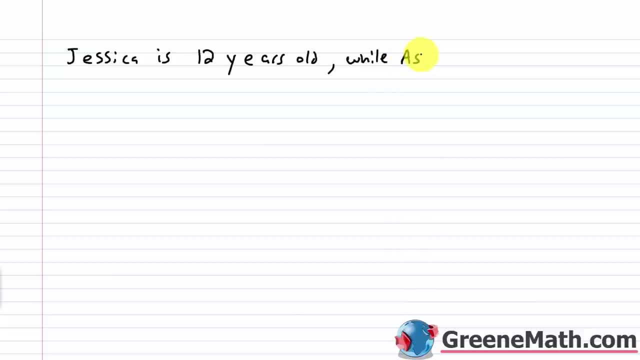 Jessica is 12 years old. While Ashley is 15 years old. 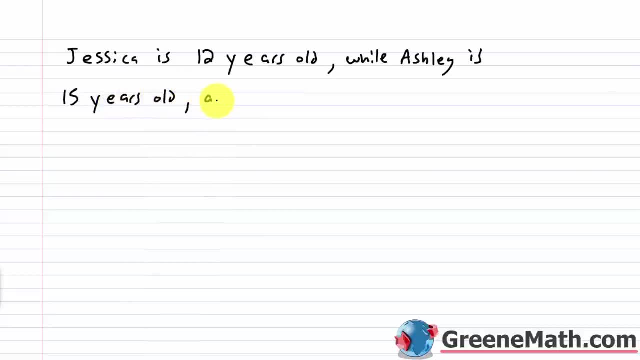 And lastly, Jennifer, she's five years younger than Jessica. Right? 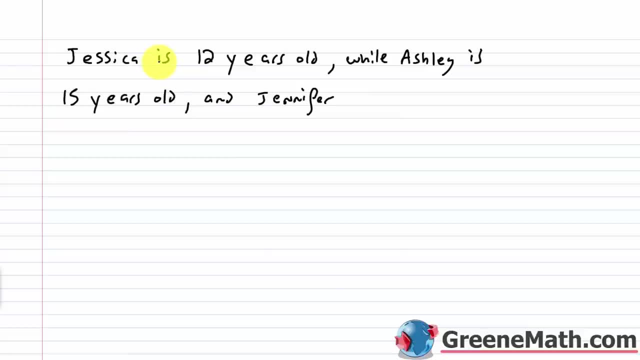 We represented her age with x minus five. So x is 12. 12 minus five is seven. And Jennifer is seven years old. So Jessica is 12 years old. 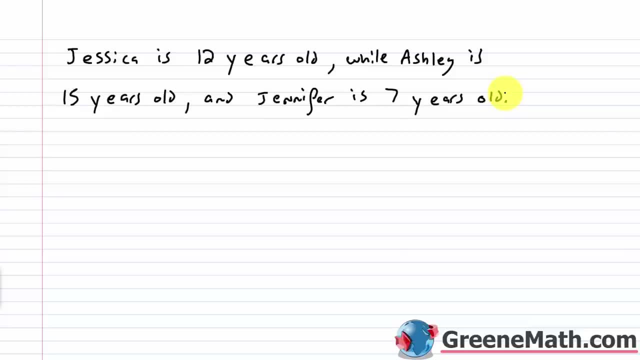 While Ashley is 15 years old. And Jennifer is seven years old. So go back to your problem and make sure that it makes sense. Make sure that the answer is reasonable. 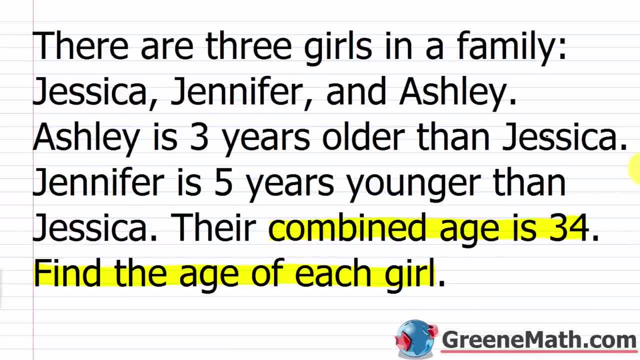 So there are three girls in a family. Jessica, Jennifer, and Ashley. Ashley is three years older than Jessica. We said Jessica was 12. So Ashley is 15. 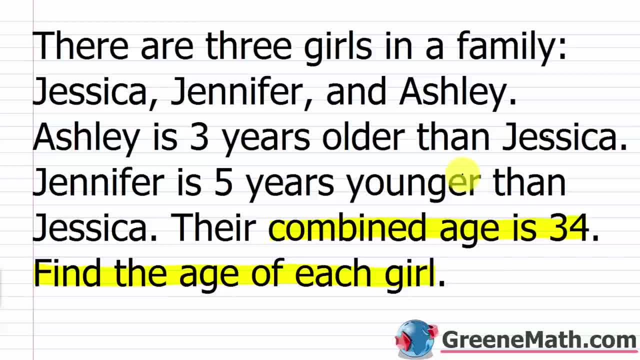 Jennifer is five years younger than Jessica. Well, we said that Jessica was 12. And so Jennifer is seven. 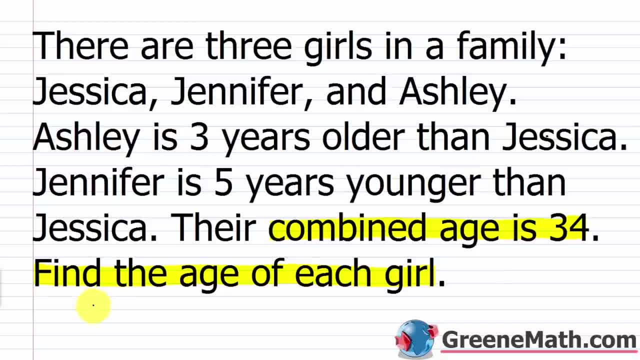 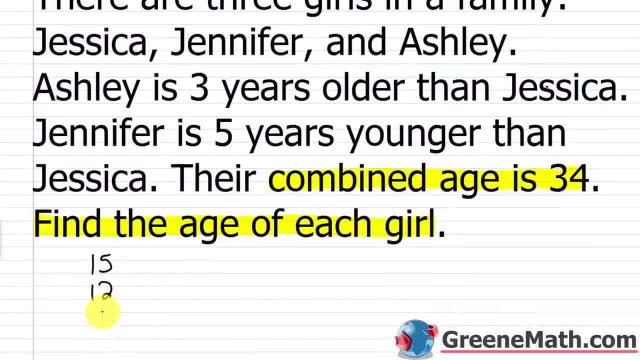 Their combined age is 34. So we have Ashley's age, which is 15. We have Jessica's age, which is 12. And we have Jennifer's age, which is seven. So if you were to sum those amounts. Five plus two is seven. 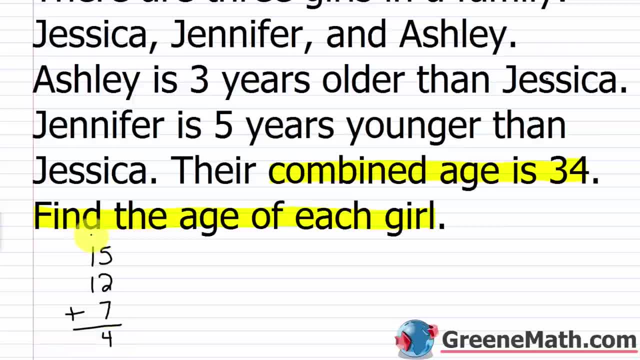 Seven plus seven is 14. Put the four down and carry a one. One plus one plus one is three. So yeah, that works out. 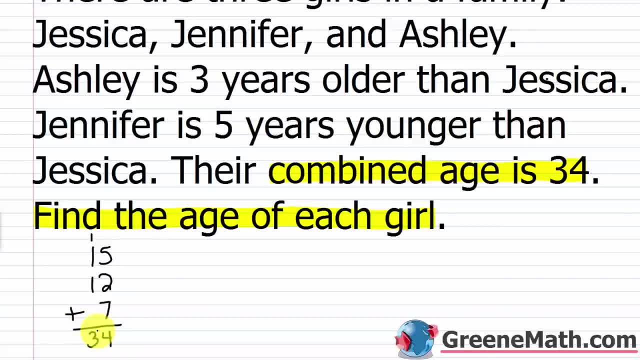 This does sum to 34. So we have the correct answer. 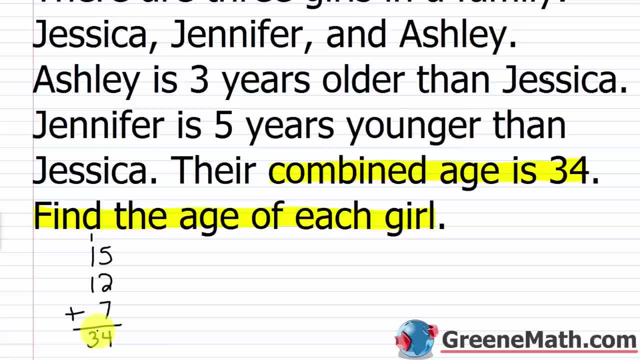 Again, Jessica is 12. Jennifer is seven. And Ashley is 15. 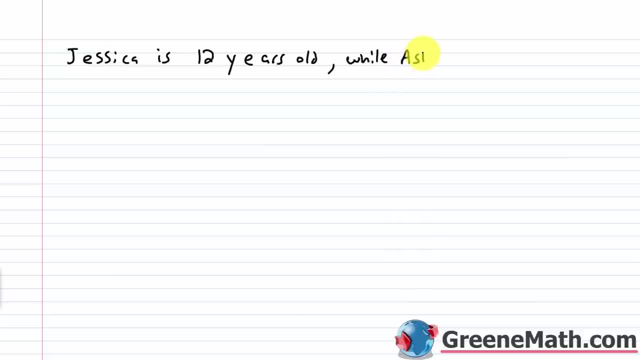 12 years old, while Ashley is 15 years old. And lastly, Jennifer. she's 5 years younger than Jessica. We represented her age with x minus 5.. So x is 12.. 12 minus 5 is 7. And Jennifer is 7 years old, So Jessica is 12 years old. 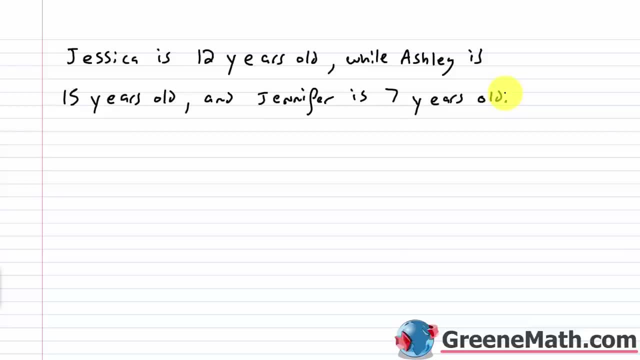 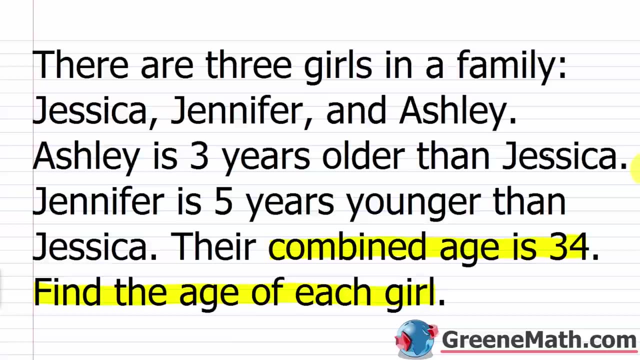 while Ashley is 15 years old and Jennifer is 7. years old. So go back to your problem and make sure that it makes sense, Make sure that the answer is reasonable. So there are three girls in a family: Jessica, Jennifer and Ashley Ashley. 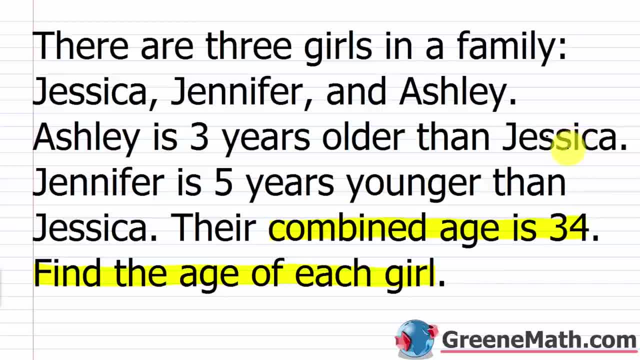 is three years older than Jessica. We said Jessica was 12,, so Ashley's 15.. Jennifer is five years younger than Jessica. Well, we said that Jessica was 12, and so Jennifer is 7.. Their combined age is 34.. So we have Ashley's age, which is 15.. We have Jessica's age, which is 12, and we have 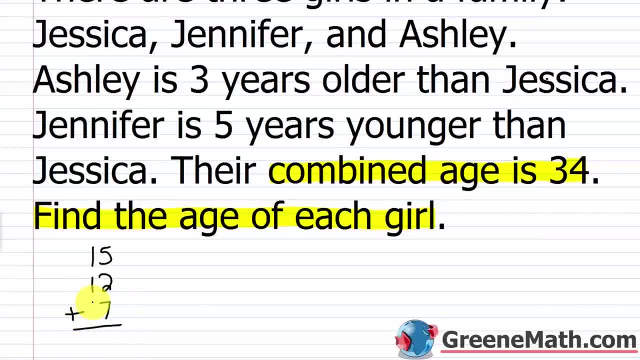 Jennifer's age, which is 7.. So if you were to sum those amounts, 5 plus 2 is 7.. 7 plus 7 is 14.. Put the 4 down, carry a 1.. 1 plus 1 plus 1 is 3.. So yeah, that works out. This does sum to 34.. 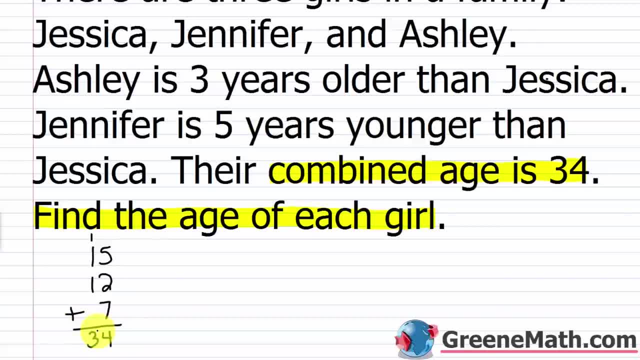 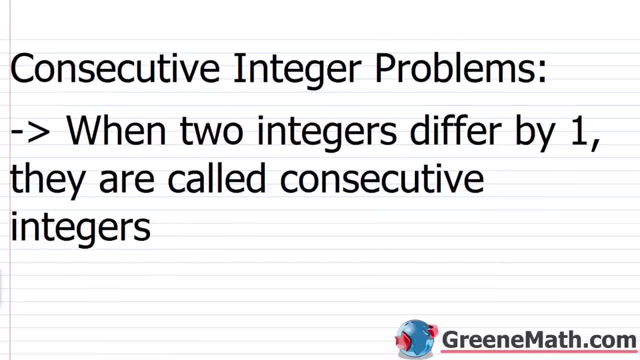 So we have the correct answer Again: Jessica is 12,, Jennifer is 7, and Ashley is 15.. All right, let's take a look at a very easy problem, to kind of conclude our introduction to applications of linear equations. So we're talking about consecutive integer problems. 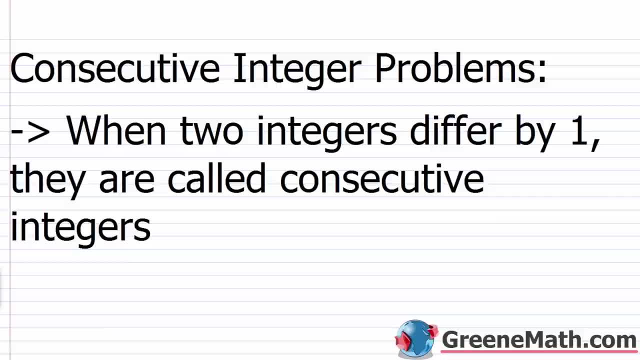 and you might see these in your book. Some books skip it because it's so easy, but basically when two integers differ by one, they are called consecutive integers. So if I have the numbers 2 and 3, they're different by one, or 14 and 15, or 123 and 124. 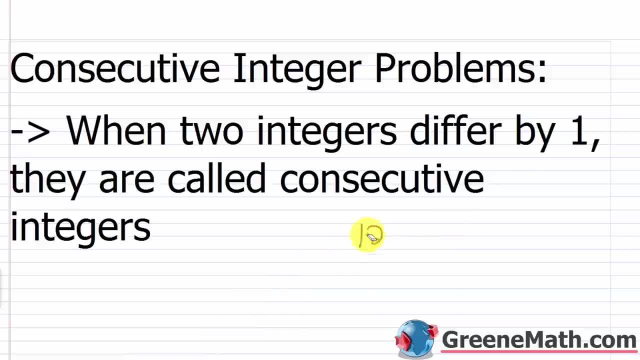 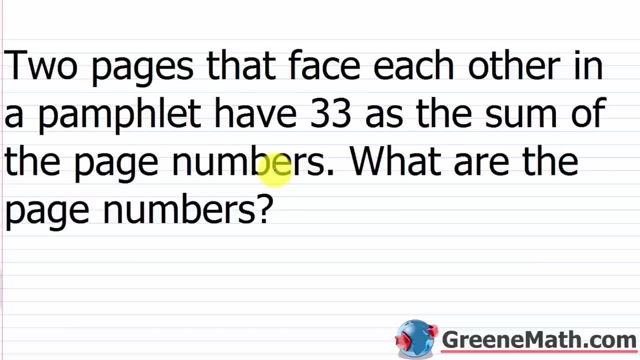 That's what we mean by consecutive integers. So let's take a look at a problem. So two pages that face each other in a pamphlet have 33 as the sum of the page numbers. What are the page numbers? So we're trying to find what are the page numbers. So this is an example of 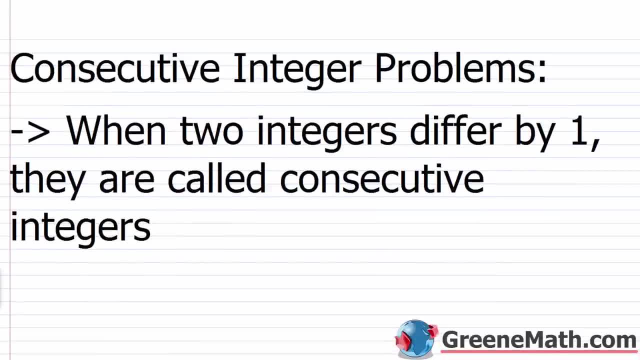 All right, let's take a look at a very easy problem to kind of conclude our introduction to applications of linear equations. 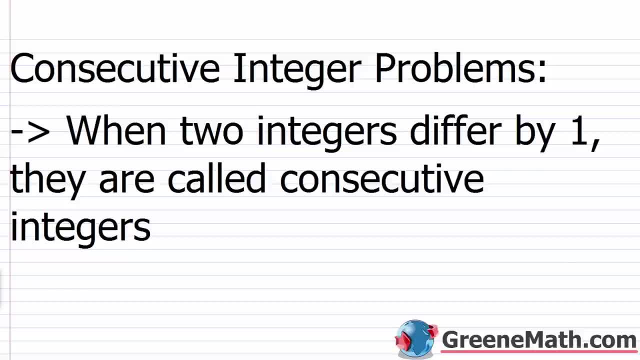 So we're talking about consecutive integer problems. And you might see these in your book. Some books skip it because it's so easy. But basically, when two integers differ by one, they are called consecutive integers. So if I have the numbers two and three, they're different by one. 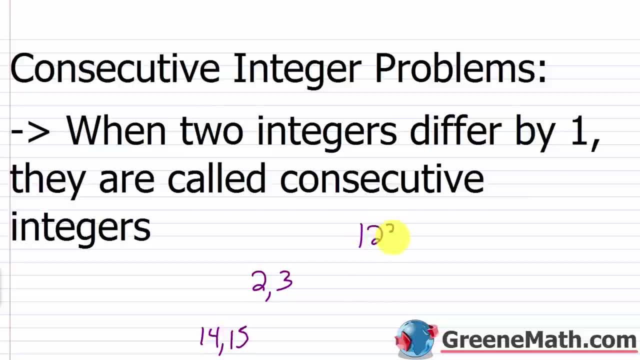 Or 14 and 15. Or 123 and 124. That's what we mean by consecutive integers. 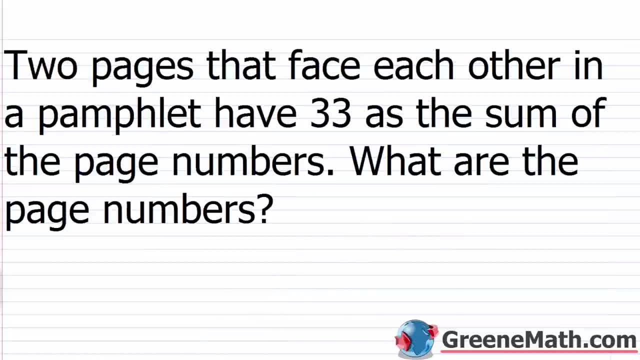 So let's take a look at a problem. So two pages that face each other in a pamphlet have 33 as the sum of the page numbers. What are the page numbers? So we're trying to find what are the page numbers. 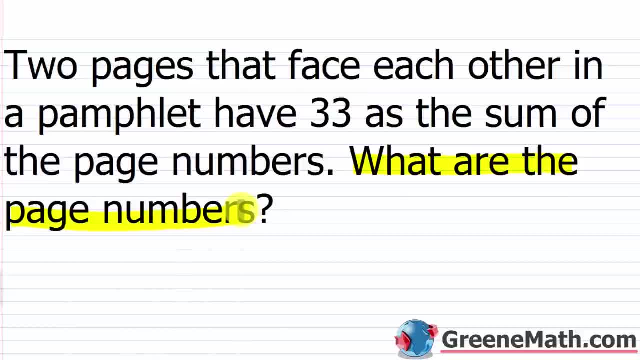 So this is an example of a consecutive integer problem. 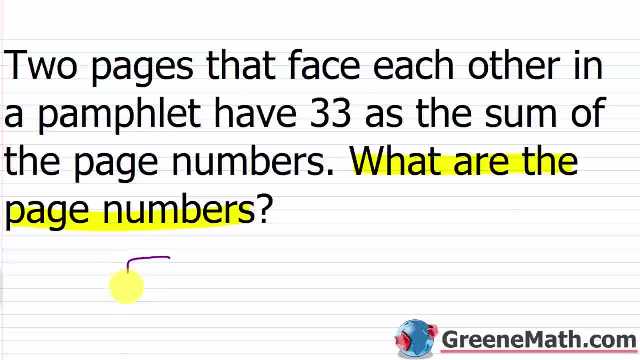 If you think about a book or pamphlet, if you have a page here, and here, and they face each other, 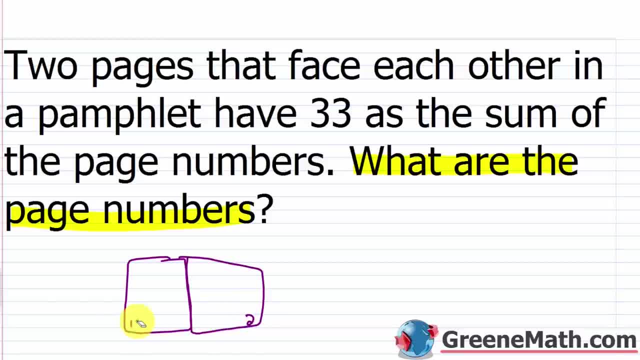 so let's say this is one and this is two. Or it could be 567 and 568. You know, so on and so forth. So we're trying to find the individual page numbers given that the sum is 33. 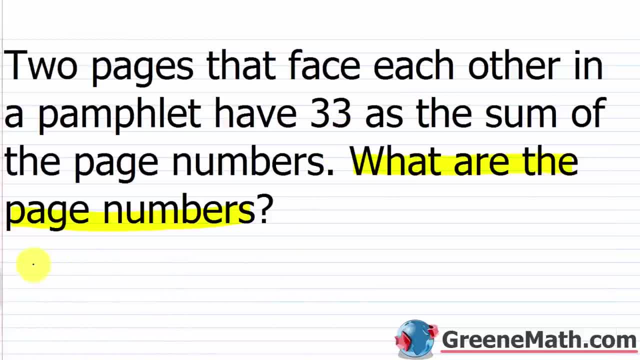 So again, just like we solved the previous two problems, we're going to let x equal one of them, one of the page numbers, and then we'll represent the other page number in terms of that variable x. 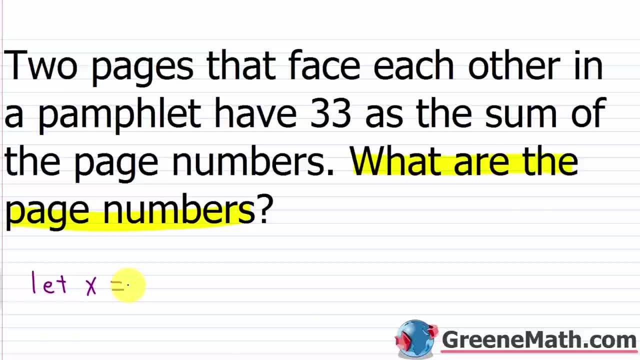 So let's let the smaller integer be x. So let x equal the smaller integer. 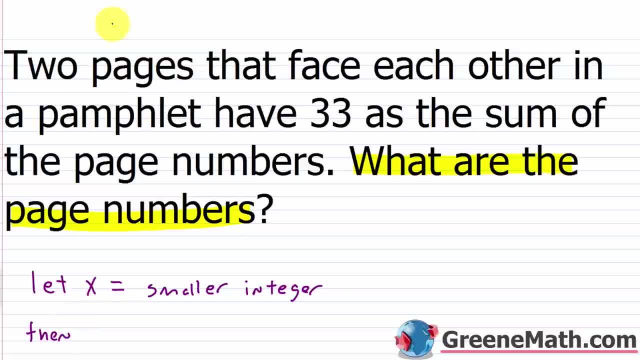 So then, since they differ by one, we could say that x plus one is equal to the larger. 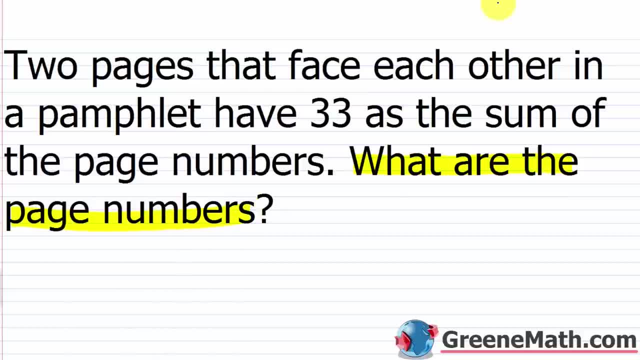 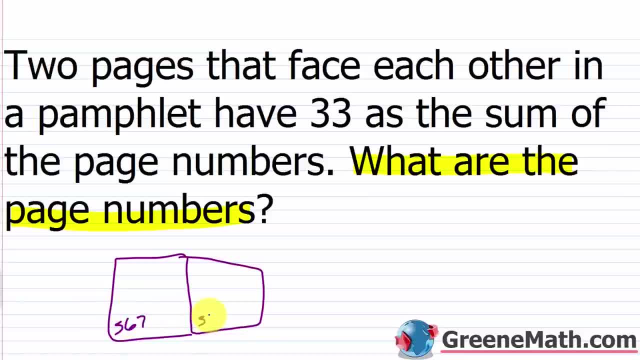 let's say 567 and 568, you know, so on and so forth. So we're trying to find the individual page numbers, given that the sum is 33.. So again, just like we saw the previous two problems, we're going to let x equal one of them, okay, one of the page numbers. 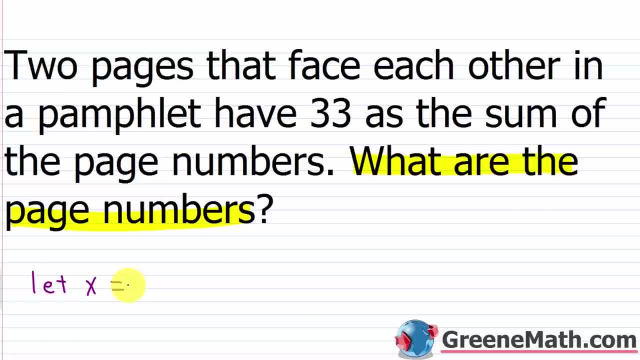 and then we'll represent the other page number in terms of that variable: x. So let's let the smaller. okay, let's let the smaller integer be x. So let x equal the smaller integer. So then, since they differ by one, we could say that x plus one is equal to the larger, the larger integer. 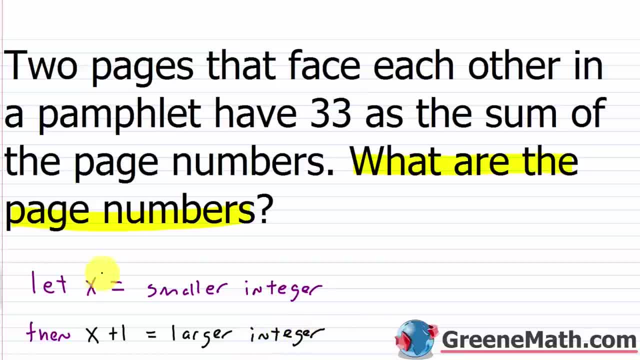 So now it's easy to set up the equation because we know that the smaller page number plus the larger page number, and I put smaller integer, larger integer, you could put smaller page number, larger page. it really doesn't matter, as long as you understand what's going on. 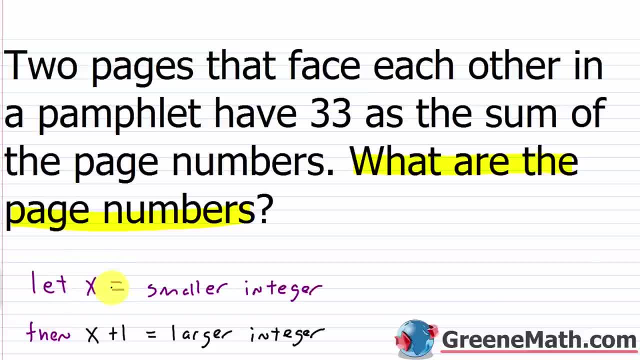 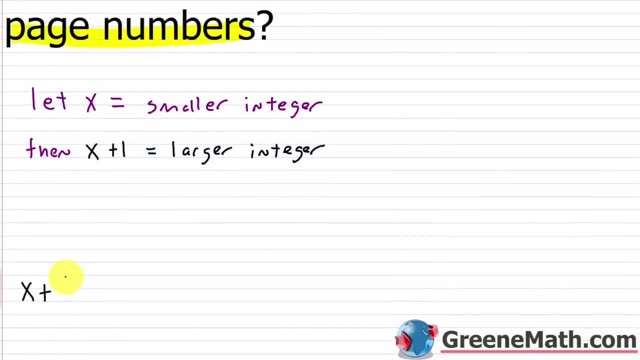 Really we're thinking that, okay, x now, which again is the smaller page number, the smaller integer plus x plus one, which is the larger page number or the larger integer, should sum to 33.. So let's go ahead and set up that equation So we would have that x plus x plus one. 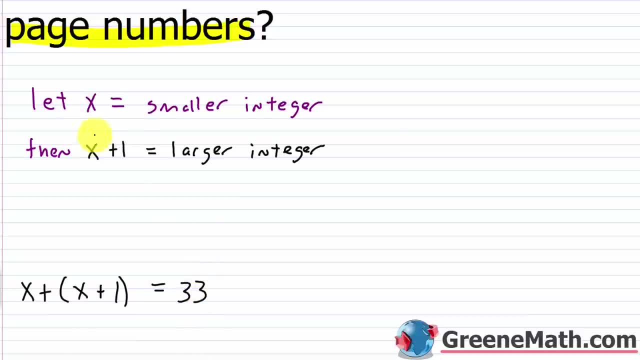 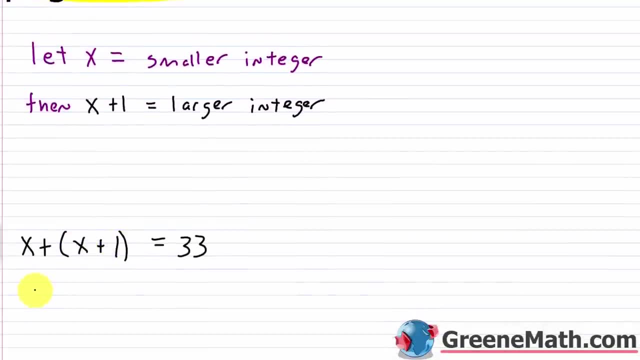 is equal to 33.. Again, this plus this gives me this: Okay, so that's my equation. So now to solve it, simplify over here. you'd have two x plus one equals 33, subtract one from both sides of the equation. 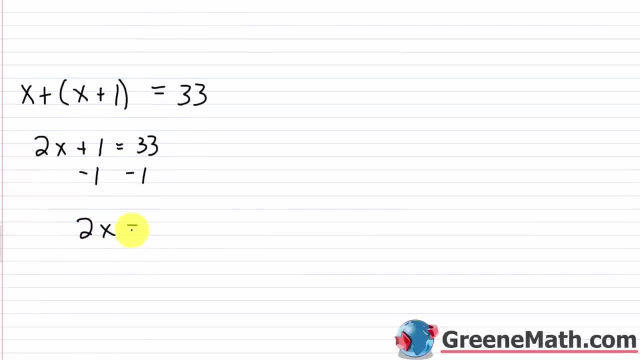 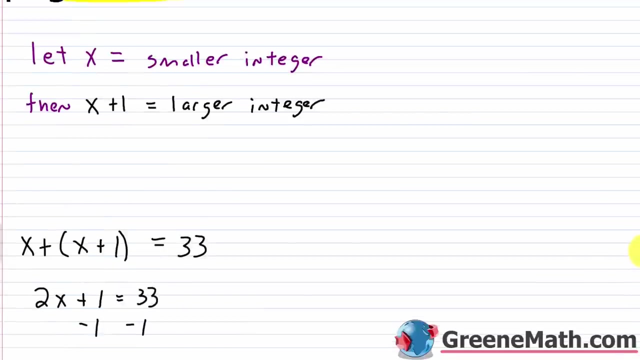 And we're going to have two. x is equal to 32.. Divide both sides of the equation by two and I'll have x is equal to 16.. So again, I'm not done. Very important that you go back up and figure out what that means. So x is the smaller integer, So that means that the smaller page. 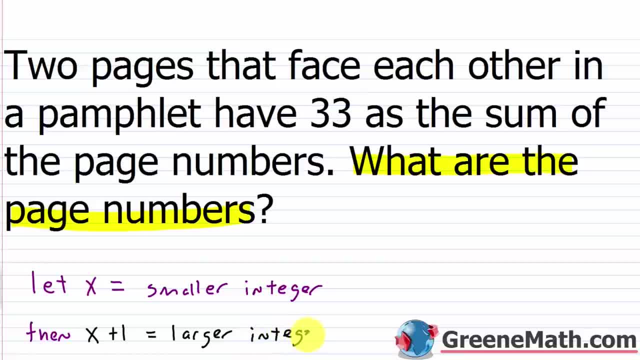 The larger integer. So now, it's easy to set up the equation because we know that the smaller page number plus the larger page number, and I put smaller integer, larger integer. You could put smaller page number, larger page. It really doesn't matter as long as you understand what's going on. Really, we're thinking that, okay, x now, which again is the smaller page number, the smaller integer, plus x plus one, which is the larger page number or the larger integer, should sum to 33. 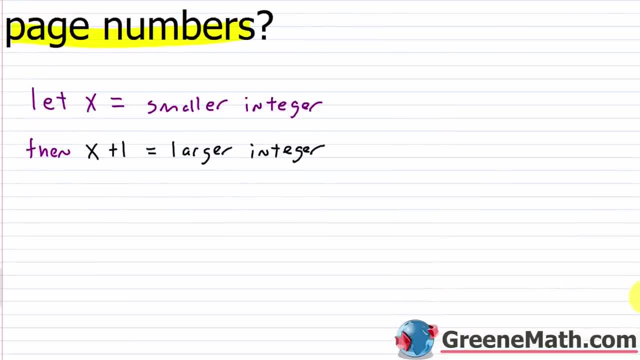 So let's go ahead and set up that equation. So we would have that x plus x plus one is equal to 33. Again, this plus this gives me this. Okay, so that's my equation. 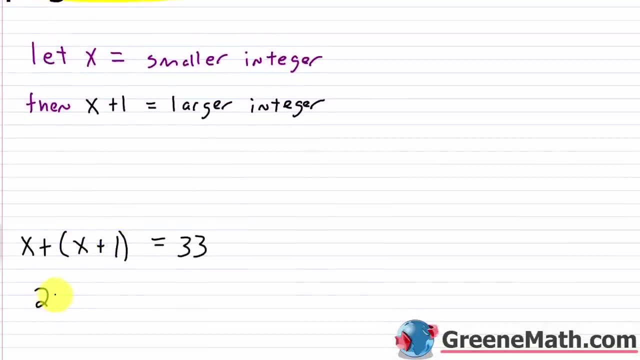 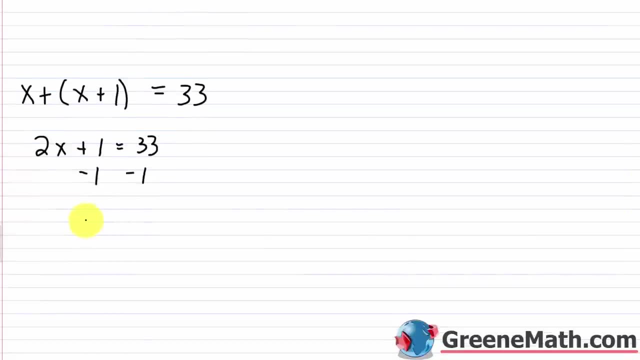 So now to solve it, simplify over here. You'd have two x plus one equals 33. Subtract one from both sides of the equation, and we're going to have two x is equal to 32. Divide both sides of the equation by one. 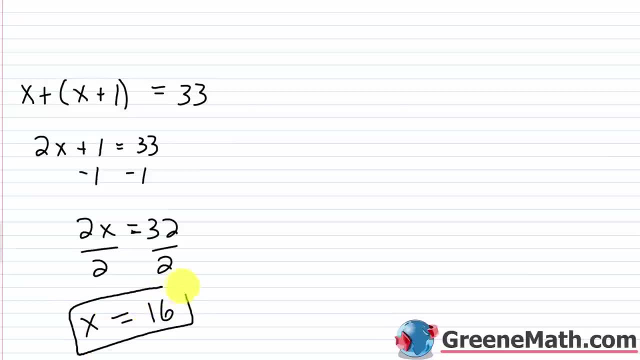 Divide by two, and I'll have x is equal to 16. So again, I'm not done. Very important that you go back up and figure out what that means. So x is the smaller integer. 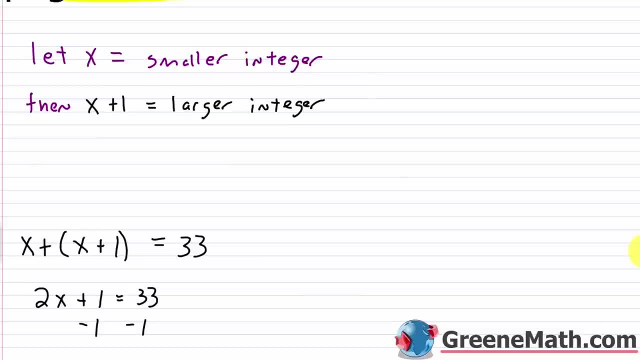 So that means that the smaller page number is 16, and the larger page number is 17. So for the page numbers, 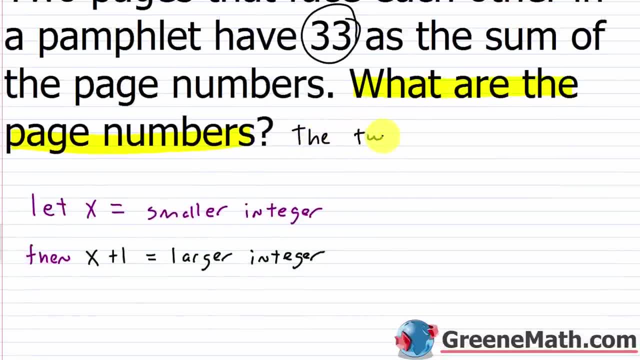 we could say that the two page numbers are 16 and 17, right? If you take 16 and you add 17, you're going to get 33, right? And the two pages do face each other in the book. 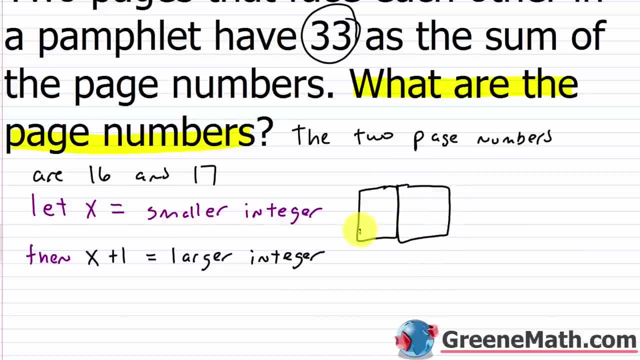 So if you had a book or pamphlet or whatever it is, this is 16, this is 17. If you close the book, the two pages would face each other. 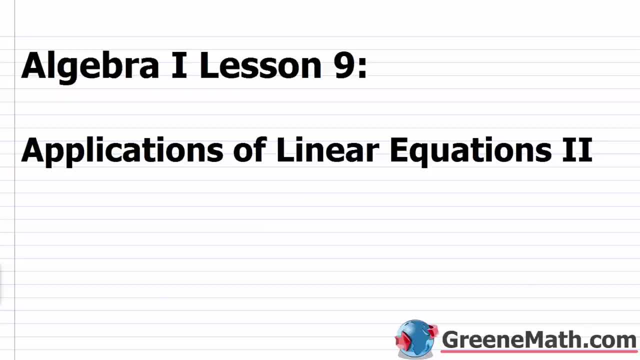 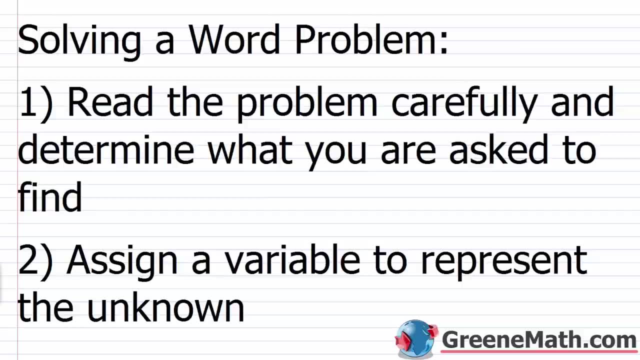 Hello and welcome to Algebra 1, Lesson 9. In this video, we're going to continue to look at applications of linear equations. So in the last lesson, we started talking about word problems. 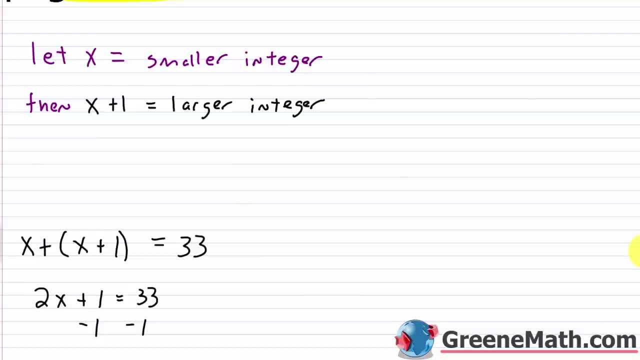 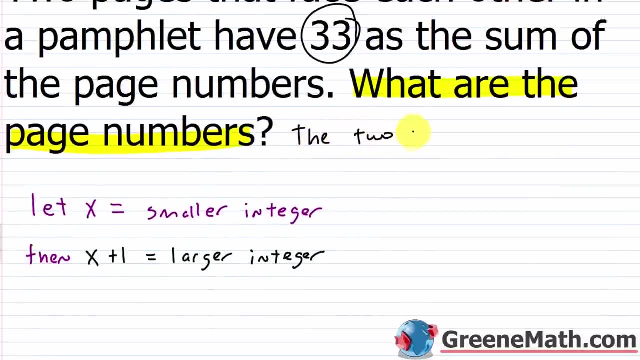 number is 16.. And the larger page number is 17.. So for the page numbers, we could say that the two page numbers are 16 and 17.. Right, If you take 16, and you add 17,, you're going to get 33,. right, And the two. 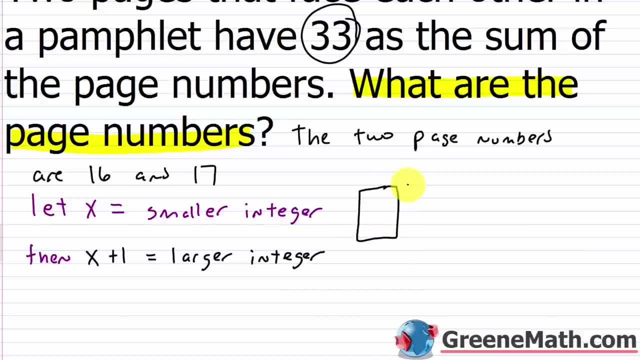 pages do face each other in the book. So if you had a book or pamphlet or whatever it is, this is 16.. This is 17.. If you close the book, the two pages would face each other. Hello and welcome. 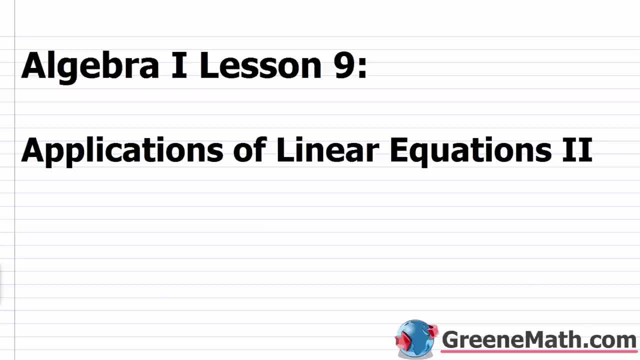 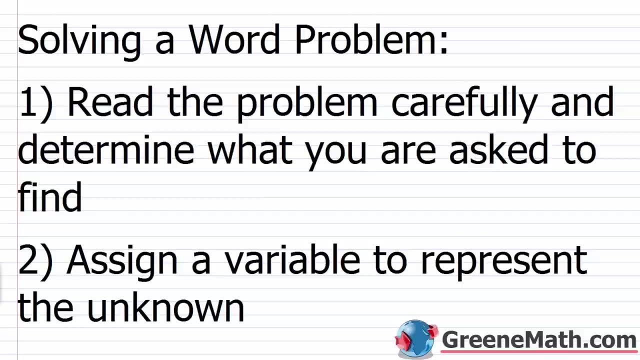 to Algebra 1, Lesson 9.. In this video we're going to continue to look at algebra 1, less than 9.. So in the last lesson we started talking about word problems And we talked about how you would go about solving a word problem. So the first thing you always want to do, you want to read. 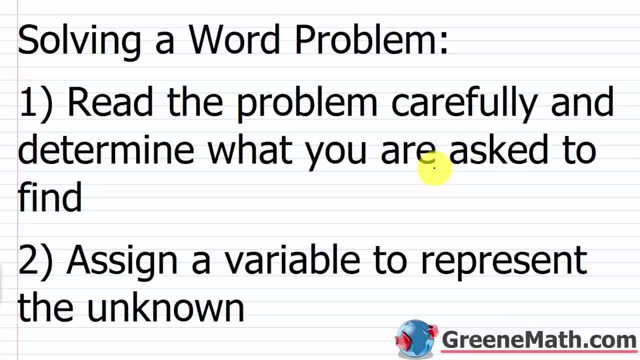 the problem carefully and determine what you're asked to find, So generally you might highlight that or write down. hey, this is what I'm looking for. That allows you to have a laser focus throughout your problem. The next thing you want to do is assign a variable to represent the unknown. 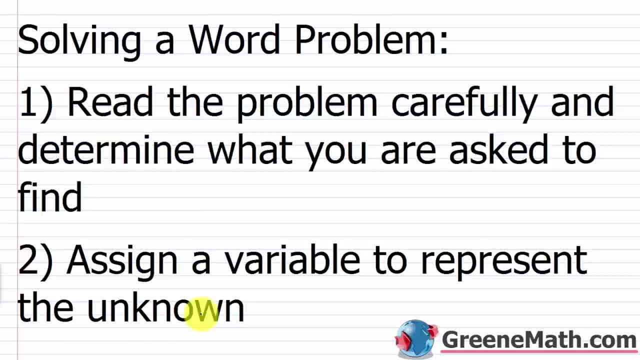 Now, in a lot of these problems, you're going to have more than one unknown, So you're going to assign a variable to represent one of the unknowns And then you're going to represent the other unknowns in terms of this variable. All right, the next thing you're going to do is write out: 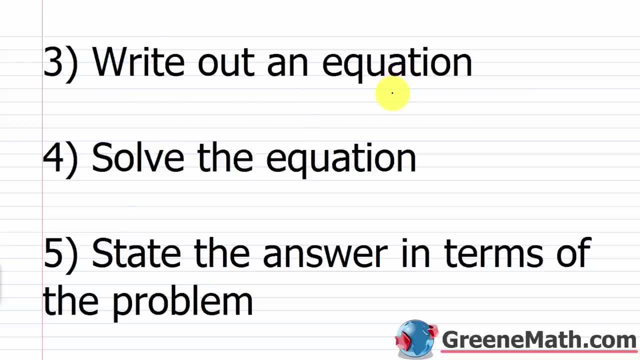 an equation And you're going to do that by reading through the problem. You'll have something equal to something else. This is going to allow you to write an equation, then solve the equation and then state the answer in terms of the problem. So that's very important. 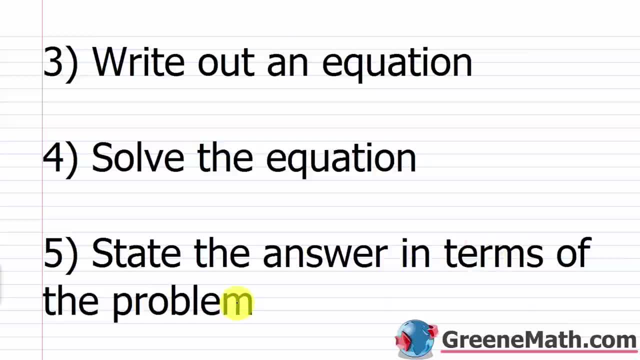 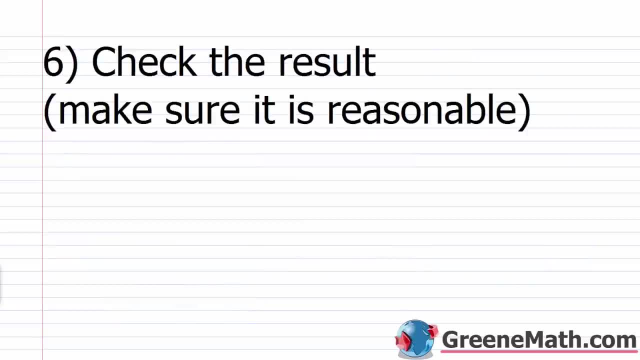 You don't just solve the equation with a word problem and then hand in your paper and say I'm done. You have to state the answer in terms of the problem And then, lastly, you want to check the result and make sure it is reasonable If you get asked for how many cars are. 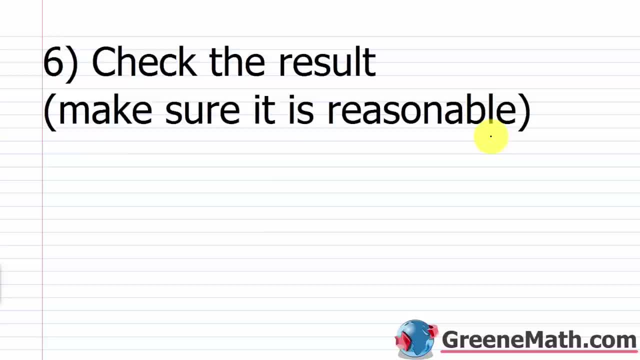 on a bridge and you get an answer that's negative. seven probably got the wrong answer right. You should have either zero or some positive amount in that scenario. So you want to make sure that your answer is reasonable. All right, so we're going to start out today by talking about everybody's. 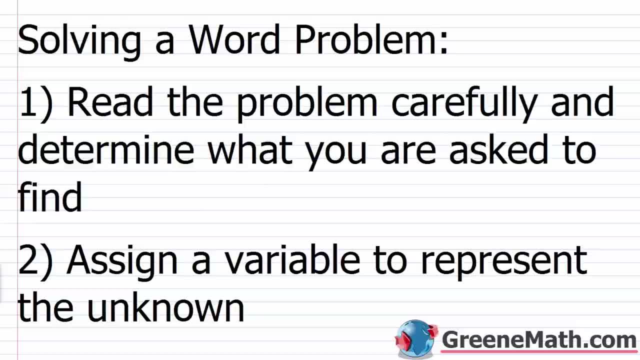 And we talked about how you would go about solving a word problem. So the first thing you always want to do, you want to read the problem carefully and determine what you are asked to find. So generally, you might highlight that or write down, hey, this is what I'm looking for. That allows you to have a laser focus throughout your problem. 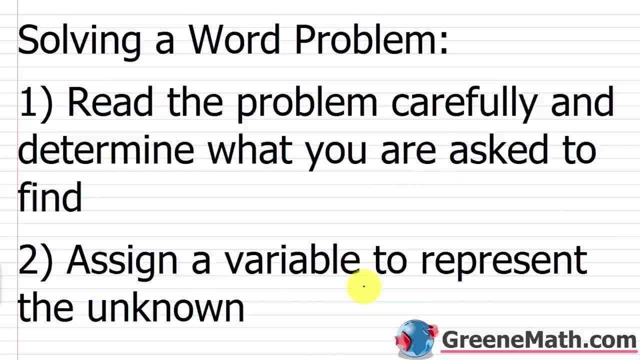 The next thing you want to do is assign a variable to represent the unknown. 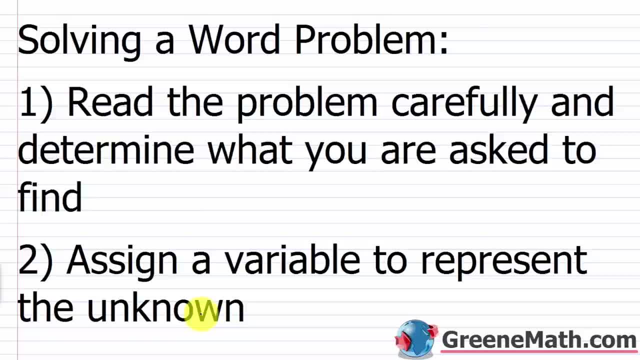 Now, in a lot of these problems, you're going to have more than one unknown. So you're going to assign a variable to represent one of the unknowns. 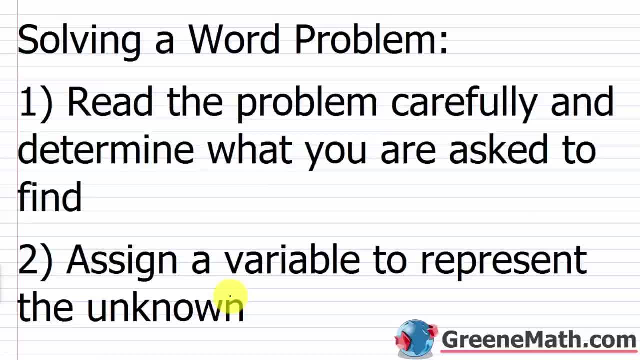 And then you're going to represent the other unknowns in terms of this variable. All right, the next thing you're going to do is write out an equation. 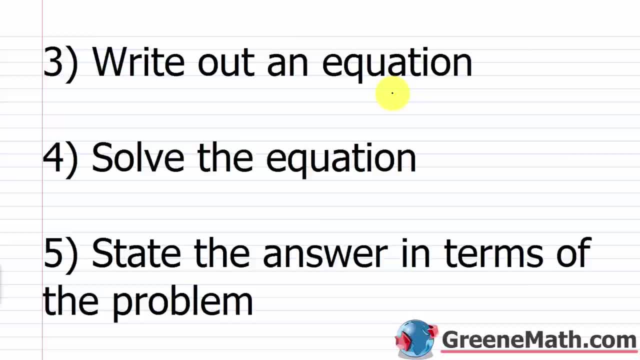 And you're going to do that by reading through the problem. You'll have something equal to something else. This is going to allow you to write an equation, then solve the equation, and then state the answer in terms of the problem. So that's very important. You don't just solve the equation with a word problem and then hand in your paper and say, I'm done. 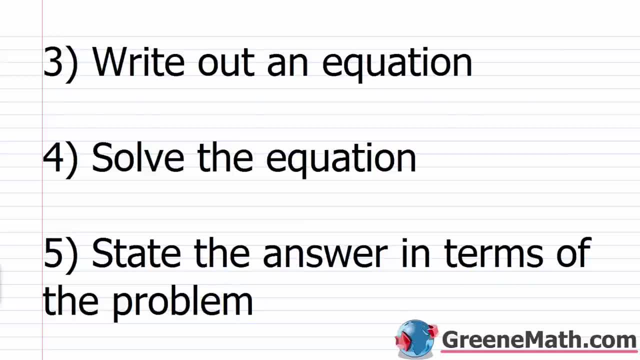 You have to state the answer in terms of the problem. And then lastly, you want to check the result and make sure it is reasonable. 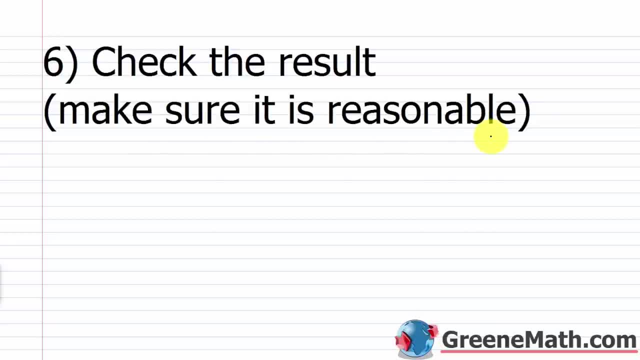 If you get asked for how many cars are on a bridge and you get an answer that's negative seven, you probably got the wrong answer, right? You should have either zero or some positive amount in that scenario. So you want to make sure that your answer is reasonable. 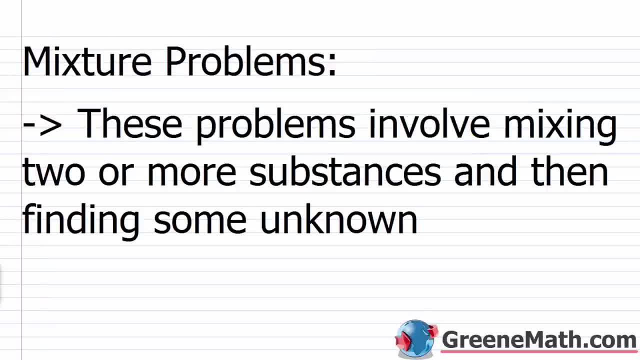 All right, so we're going to start out today by talking about everybody's favorite, which you will come to know as mixture problems. 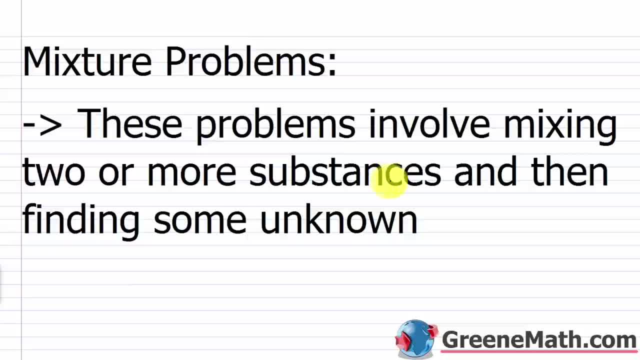 So these problems involve mixing two or more substances and then finding some unknown. Now, the problems we're going to look at today 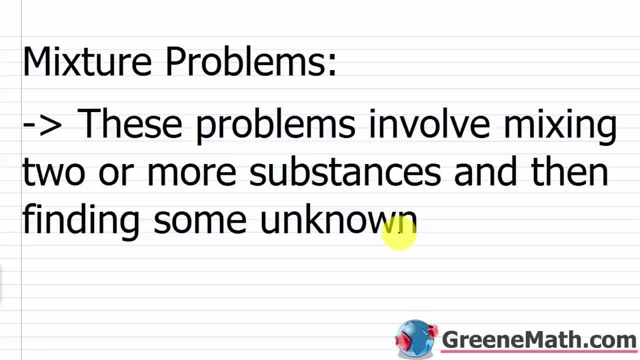 are going to be relatively simple, but as we move forward, they're going to get more and more complex. 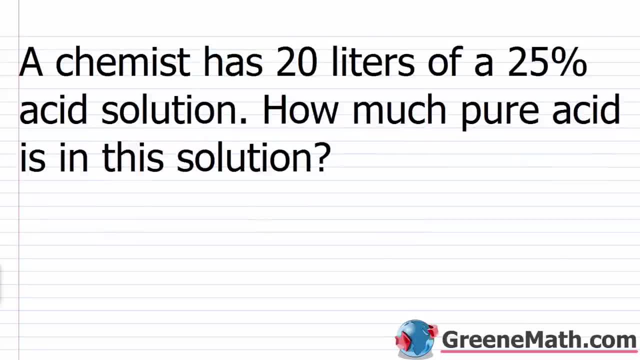 So the first thing we need to understand with a mixture problem is how to find the pure amount of a substance in a mixture. 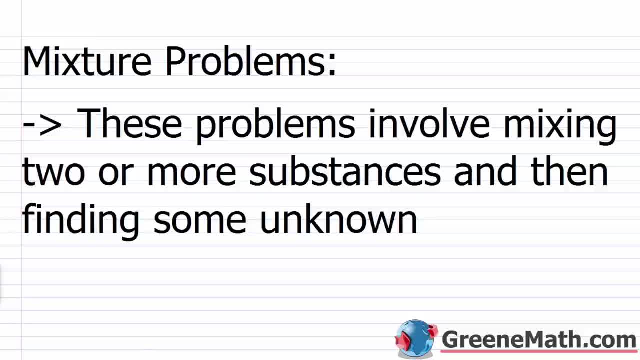 favorite, which you will come to know them as mixture problems. So these problems involve mixing two or more substances and then finding some unknown. Now, the problems we're going to look at today are going to be relatively simple, But as we move forward they're going to get more. 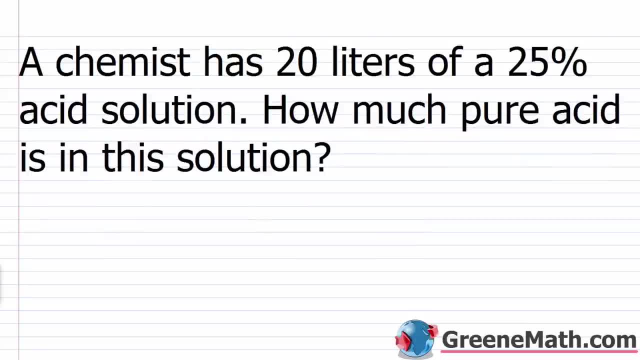 and more complex. So the first thing we need to understand with a mixture problem is how to find the pure amount of a substance in a mixture. So here's a quick example. So a chemist has 20 liters of a 25% acid solution. So what does that mean? when I say a 25% acid solution, It means 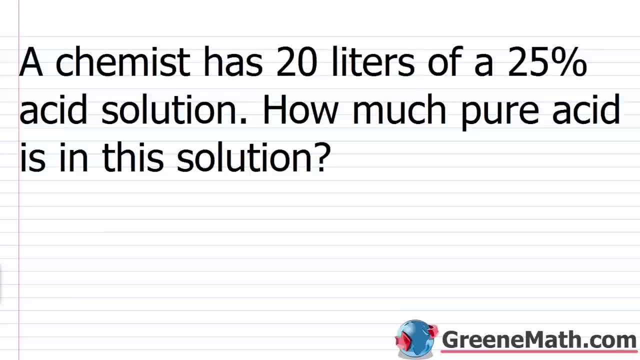 that 25% of it is acid. How much pure acid is in this solution? So to figure this out, you just take the amount of the solution, which is 20 liters. So I'm just going to write 20.. I don't need to. 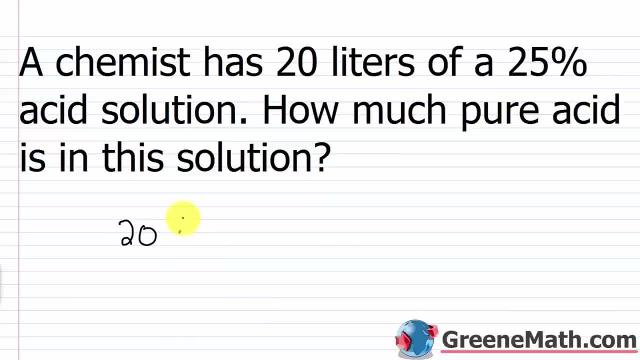 write liters there And I would multiply it by the percentage of acid that's in it. So if it's Now, I'm going to convert 25% to a decimal, So that's 0.25.. And this will tell me how much pure. 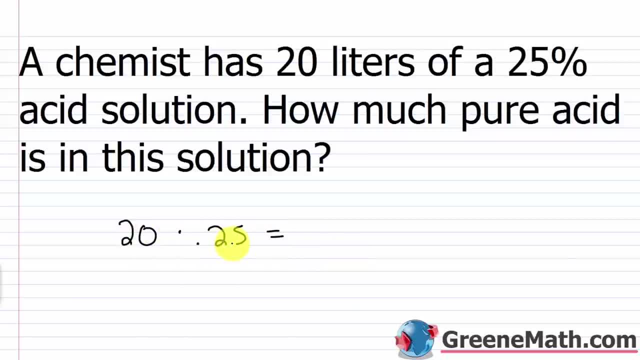 acid is in the solution. So 20 times 0.25 is the same as 20 times 1. fourth, And I can do that in my head That's going to be five. It's basically like taking 20 and dividing by four, So there. 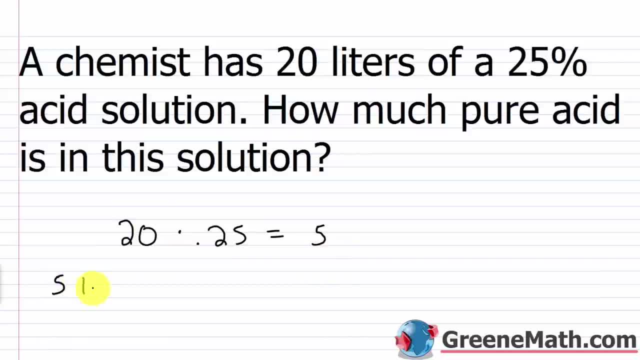 would be five liters. five liters of pure acid, That's 20 liters of a 25% acid solution. So how much pure acid is in the solution? Again, 25% of 20 is five. So that means there's five liters of pure acid. All right, we're going to. 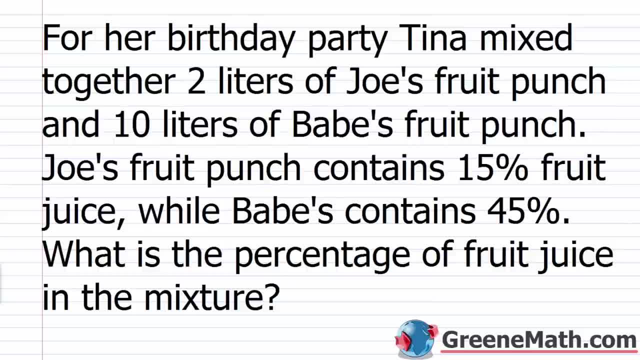 look at another one that's simple and kind of gives us a little warm up as far as you know, understanding how to find the pure amount of something Okay, very, very important. So this won't be a typical mixture problem. This will be a very easy one. 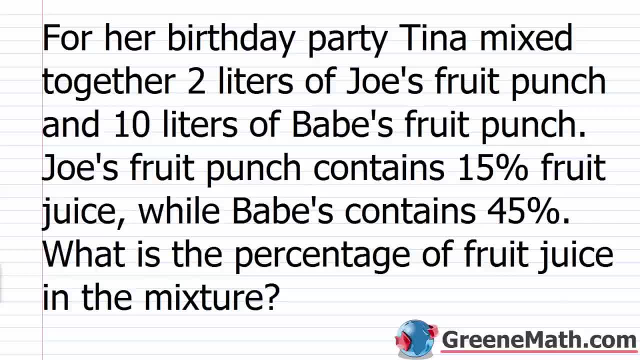 So for her birthday party, Tina mixed together two liters of Joe's Fruit Punch and 10 liters of Babe's Fruit Punch. Joe's Fruit Punch contains 15% fruit juice, while Babe's contains 45%. What is the percentage of fruit juice in the mixture? So what is the percentage? 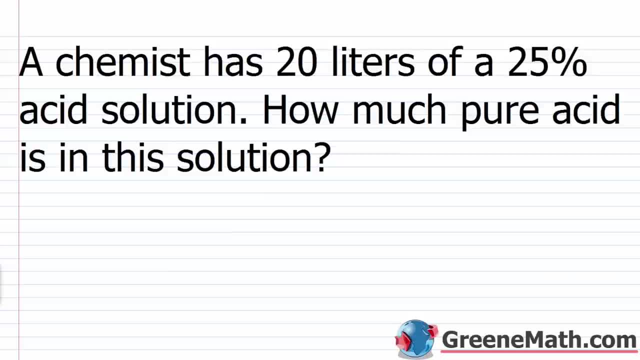 So here's a quick example. So a chemist has 20 liters of a 25% acid solution. 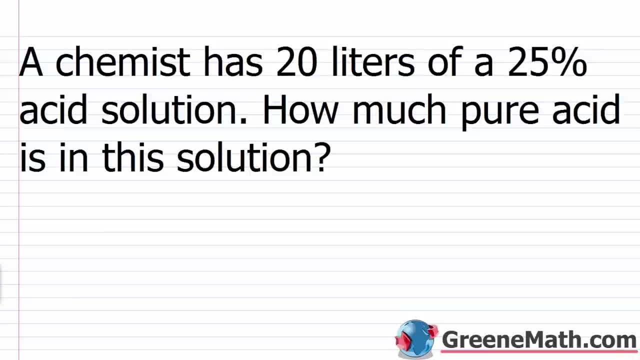 So what does that mean when I say a 25% acid solution? It means that 25% of it is acid. 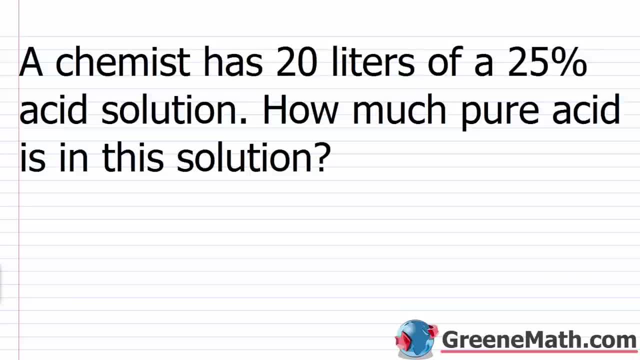 How much pure acid is in this solution? So to figure this out, you just take the amount of the solution, which is 20 liters. 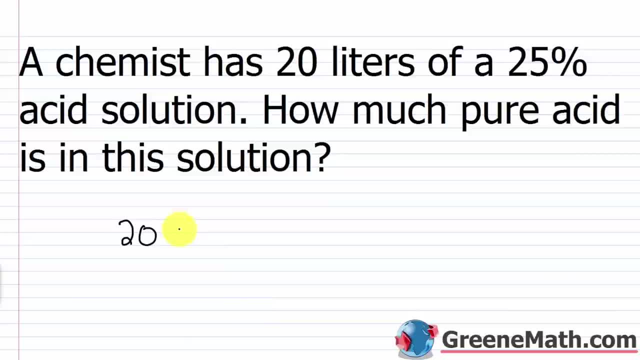 So I'm just going to write 20. I don't need to write liters there. And I would multiply it by the percentage of acid that's in it. So if it's a 25% acid solution, 25% of it is acid. Now, I'm going to convert 25% to a decimal. So that's 0.25. 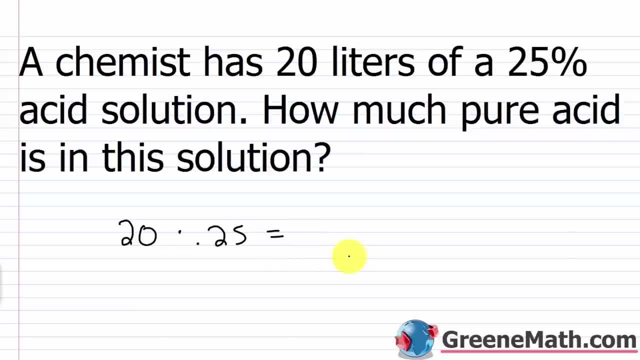 And this will tell me how much pure acid is in the solution. 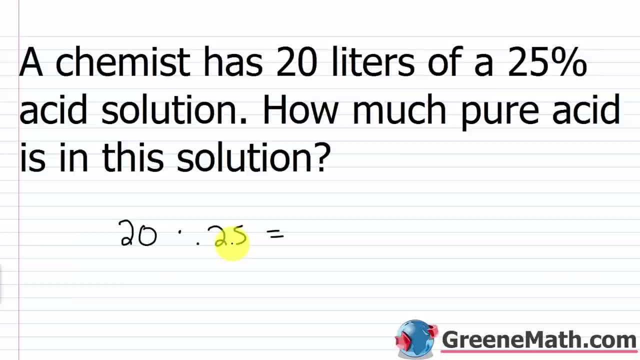 So 20 times 0.25 is the same as 20 times 1 4th. And I can do that in my head. 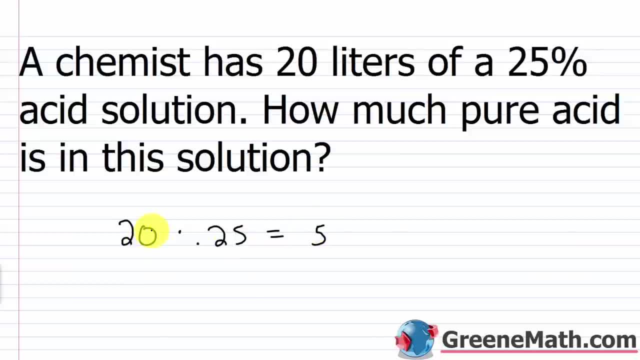 That's going to be 5. It's basically like taking 20 and dividing by 4. 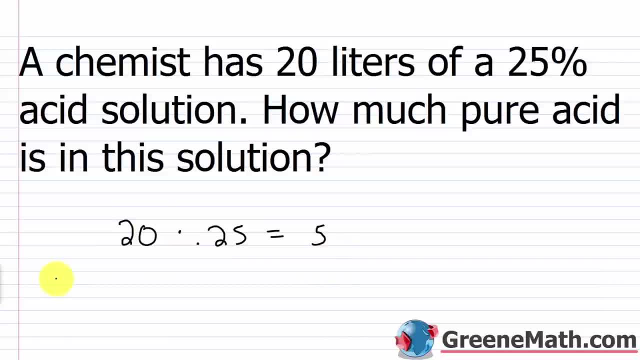 So there would be 5 liters, 5 liters of pure acid. 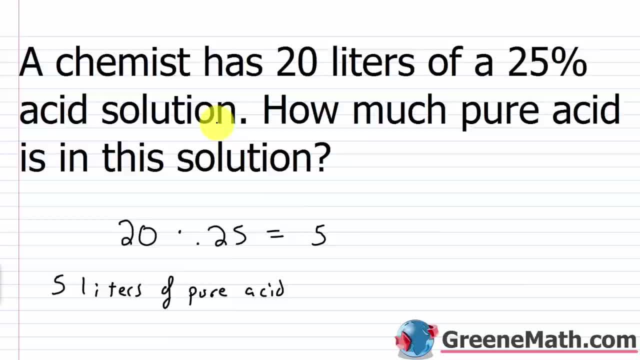 It's 20 liters of a 25% acid solution. So how much pure acid is in the solution? 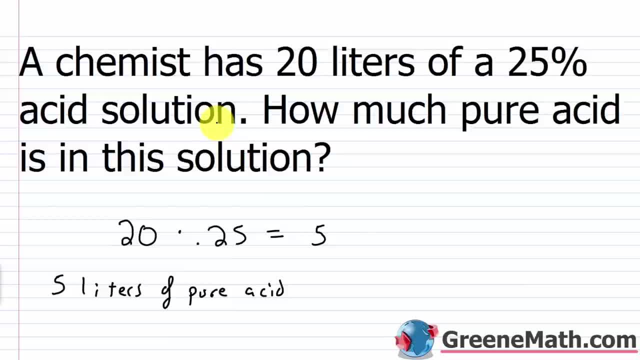 Again, 25% of 20 is 5. So that means there's 5 liters of pure acid. 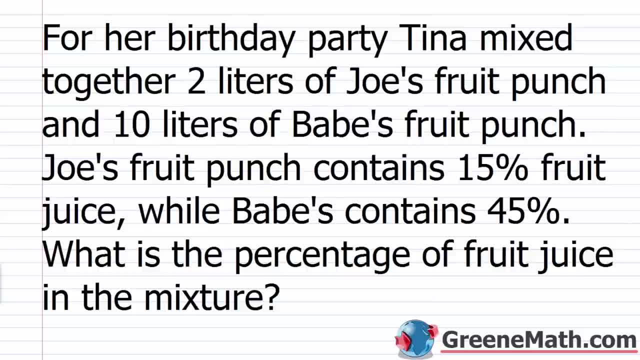 We're going to look at another one that's simple and kind of gives us a little warm up as far as, you know, understanding how to find the pure amount of something. Very, very important. So this won't be a typical mixture problem. This will be a very easy one. 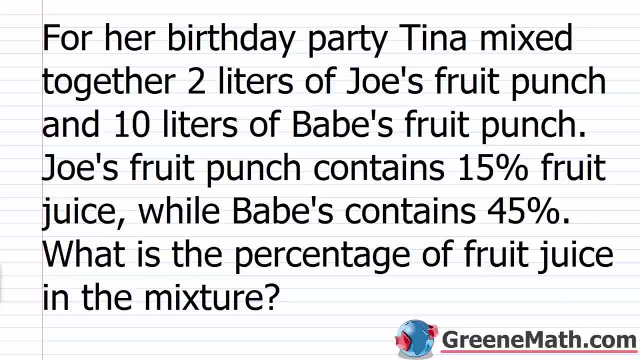 So for her birthday party, Tina mixed together 2 liters of Joe's Fruit Punch and 10 liters of Babe's Fruit Punch. 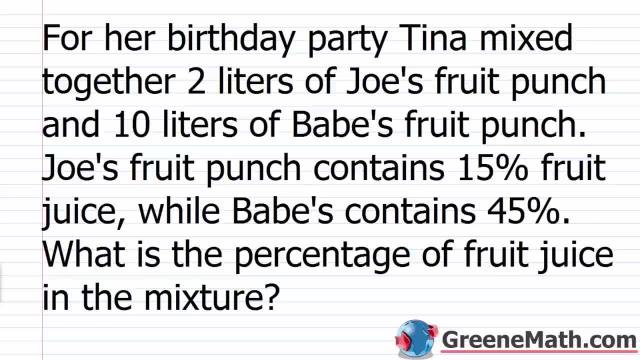 Joe's Fruit Punch contains 15% fruit juice while Babe's contains 45%. What is the percentage of fruit juice in the mixture? So what is the percentage 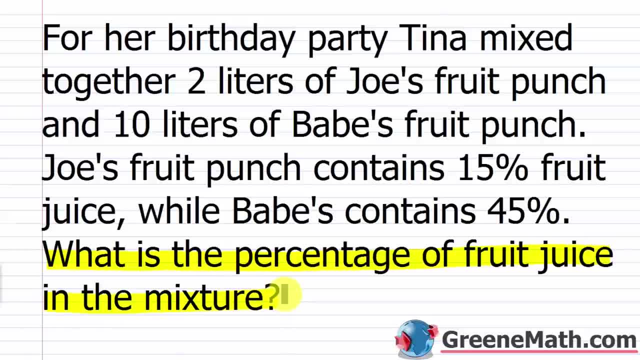 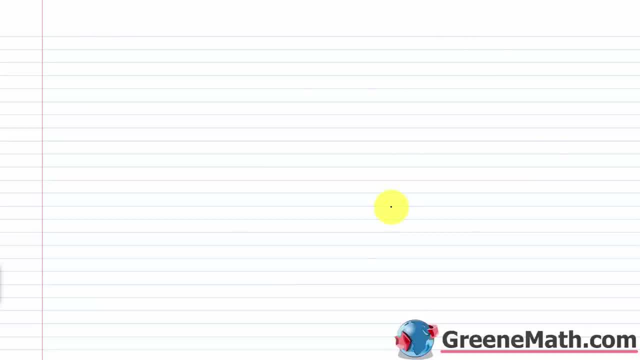 of fruit juice in the mixture. How do I obtain that? Forget about the numbers, for now. If I want the percentage of something, well, I would want The amount that I'm looking for as a pure amount over the total. So in this particular case, 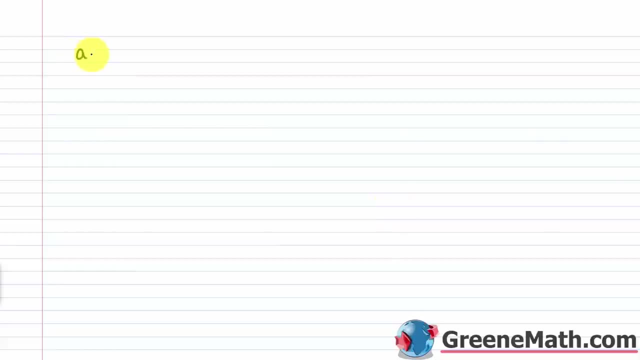 we're looking for the amount of pure fruit juice. So the amount of pure fruit juice- and that's going to be in liters, right, Because we're talking about this- mixtures in terms of liters over just the amount of the mixture, the amount. 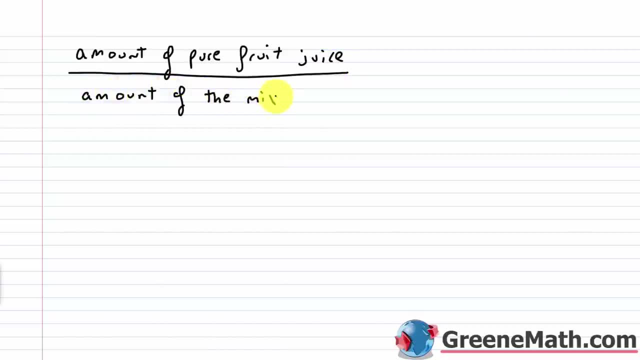 of the mixture, And we know that this amount here, the amount of the mixture, is larger and this amount is smaller, So we're going to end up with something that's less than one, greater than zero, right? It's going to be a decimal, something like point something. Now I would then take that amount and I 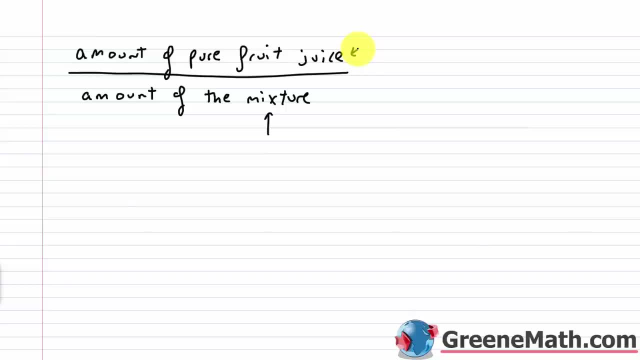 would convert it to a percentage, And then I could say, hey, this is the percentage of fruit juice in this mixture. So let's fill in the information here. How much pure fruit juice do we have? Well, we have two liters of Joe's fruit punch and 10 liters of Babes. So we have two liters. 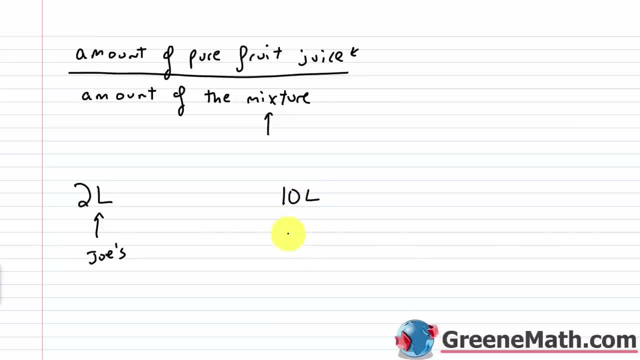 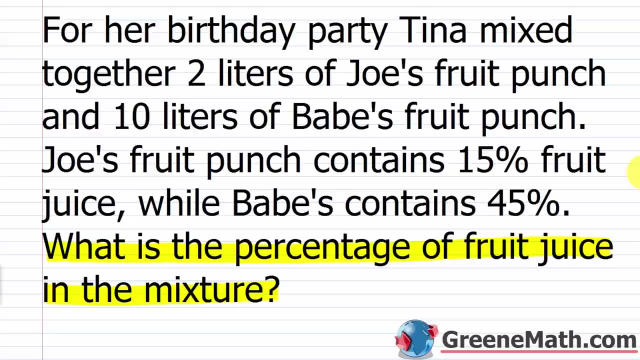 This is Joe's, and we have 10 liters of Babes. Now I can already figure out what the total amount of the mixture is going to be, because two liters plus 10 liters is 12 liters, So I'm just going to write 12.. Now what's the concentration of each? Well, it says that Joe's fruit punch is 15% fruit juice. 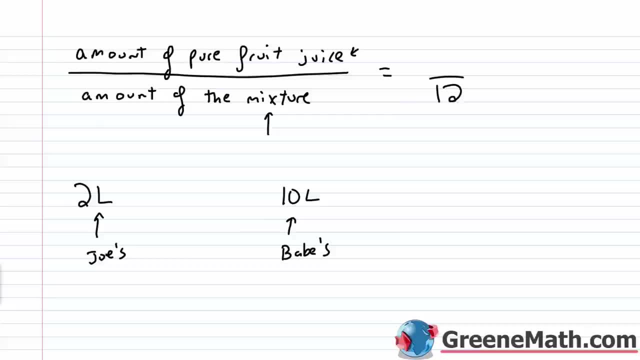 And Babes is 45%. So Joe's is 15%, 15% and Babes is 45%. So if I multiply two, which is the number of liters of Joe's times 15% or 0.15, in decimal form, that would give me the amount of pure fruit. 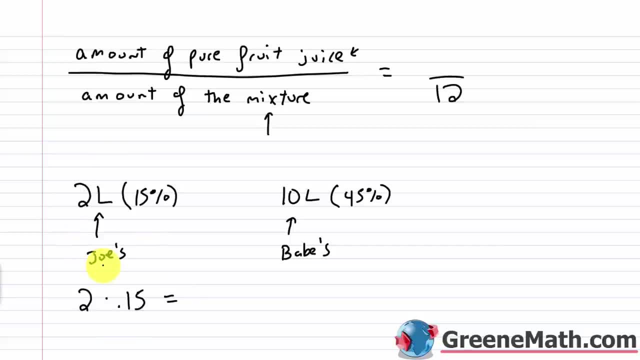 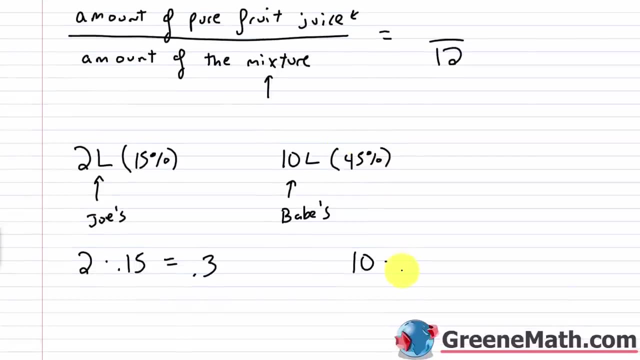 juice in Joe's fruit punch right Added from that. So two times 0.15 is 0.3. Then if I do the same thing over here, if I have 10, which is the number of liters from the Babes fruit punch- times 0.45,, which is 45% as a decimal. of fruit juice in the mixture? How do I obtain that? Forget about the numbers for now. 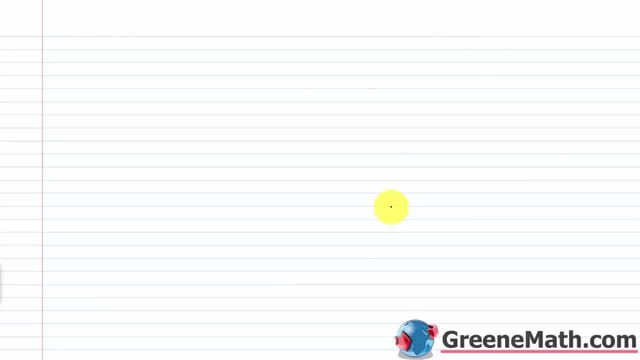 If I want the percentage of something, well, I would want 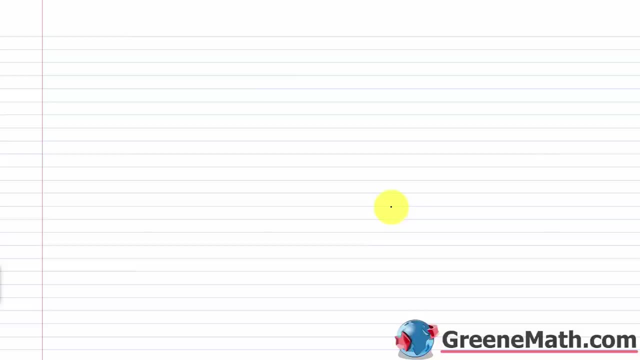 the amount that I'm looking for as a pure amount over the total. 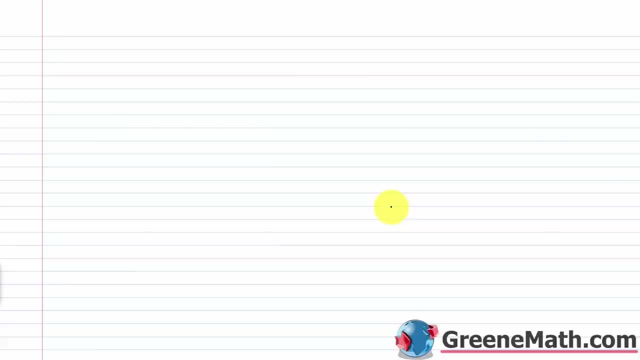 So in this particular case, we're looking for the amount of pure fruit juice. So the amount of pure fruit juice and that's going to be in liters, right? Because we're talking about this mixture is in terms of liters over just the amount of the mixture. 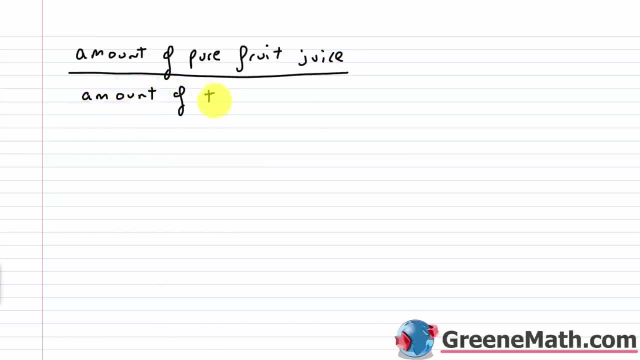 The amount of the mixture. 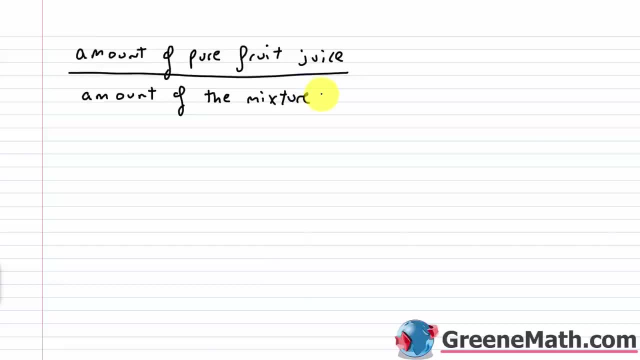 And we know that this amount here, the amount of the mixture is larger and this amount is smaller. 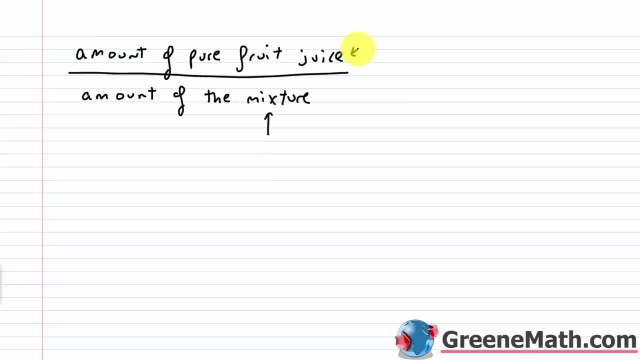 So we're going to end up with something that's less than one greater than zero, right? It's going to be a decimal, something like point something. 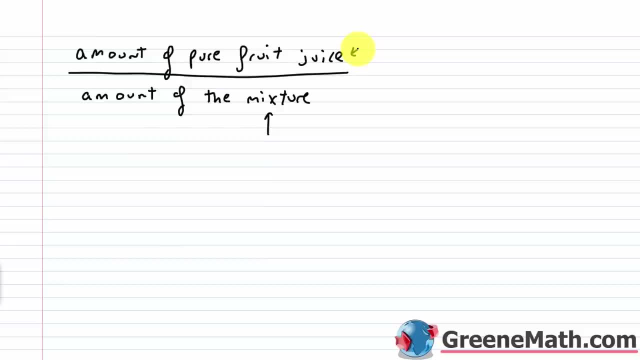 Now I would then take that amount and I would convert it to a percentage. And I can say, hey, this is the percentage of fruit juice in this mixture. 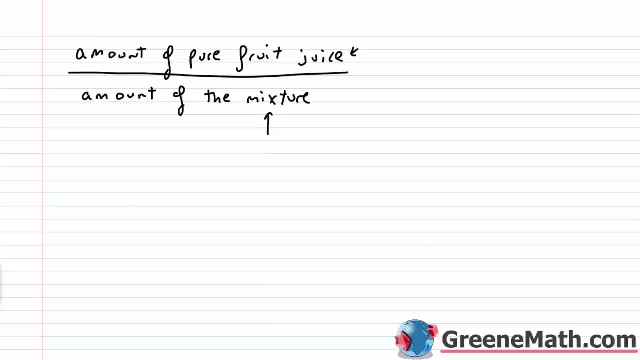 So let's fill in the information here. How much pure fruit juice do we have? Well, we have two liters of Joe's Fruit Punch and 10 liters of Babes. 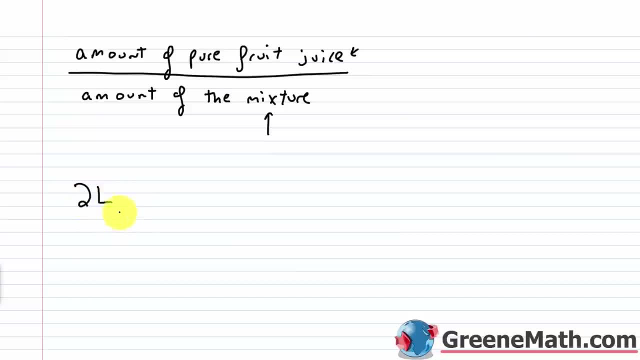 So we have two liters. This is Joe's. And we have 10 liters of Babes. Now I can already figure out what the total amount of the mixture is going to be because two liters plus 10 liters is 12 liters. So I'm just going to write 12. Now, what's the concentration of each? 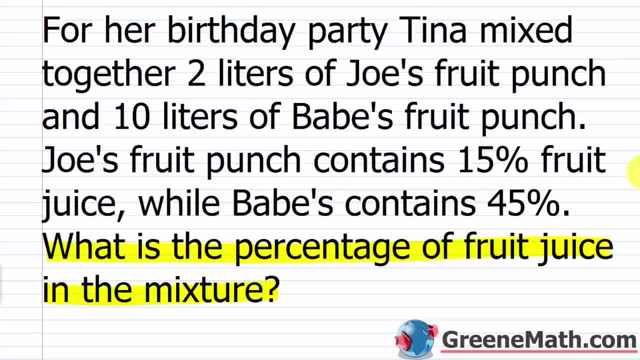 Well, it says that Joe's Fruit Punch is 15% fruit juice and Babes is 45%. 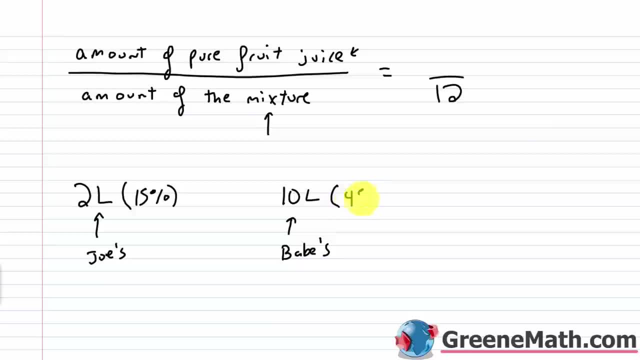 15% and Babes is 45%. 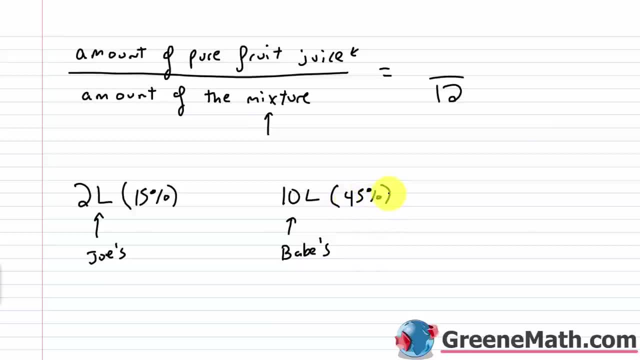 So if I multiply two, which is the number of liters of Joe's times 15% or 0.15 in decimal form, that would give me the amount of pure fruit juice in Joe's Fruit Punch, right? The amount I added from that. 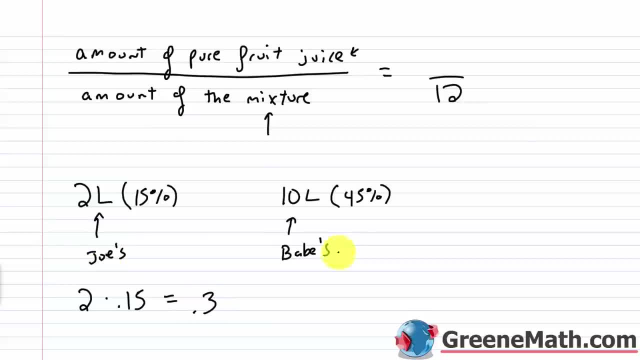 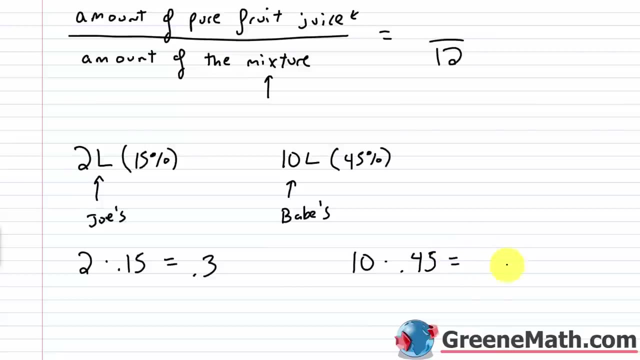 So two times 0.15 is 0.3. Then if I do the same thing over here, if I have 10, which is the number of liters from the Babes Fruit Punch times 0.45, which is 45% as a decimal, that's going to give me the amount of pure fruit juice that I'm throwing in from Babes Fruit Punch. 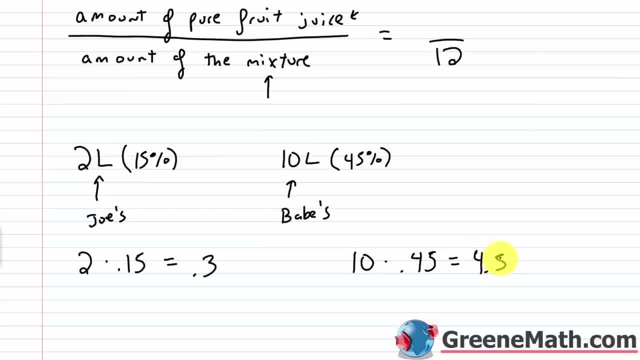 So this is going to be 4.5. So, 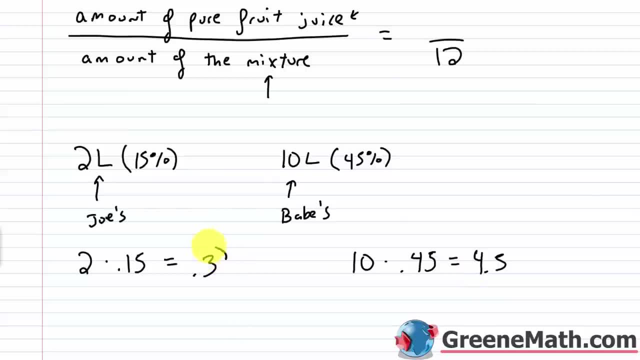 if I sum these two amounts together, the amount of pure fruit juice that I'm putting in from Joe's plus the amount of pure fruit juice that I'm putting in from Babes, I'd get 4.8, right? 0.3 plus 4.5 is 4.8. So essentially I have 4.8 divided by 12. 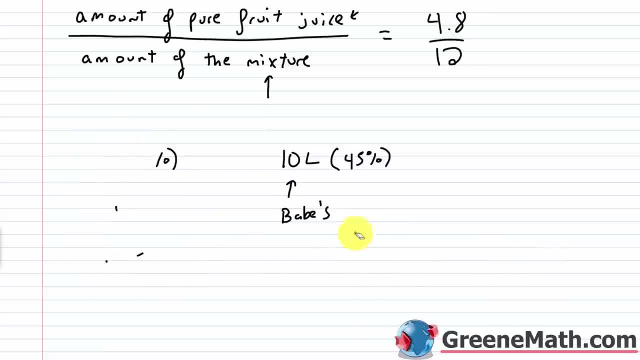 So let's erase this real quick. We'll do our calculation. 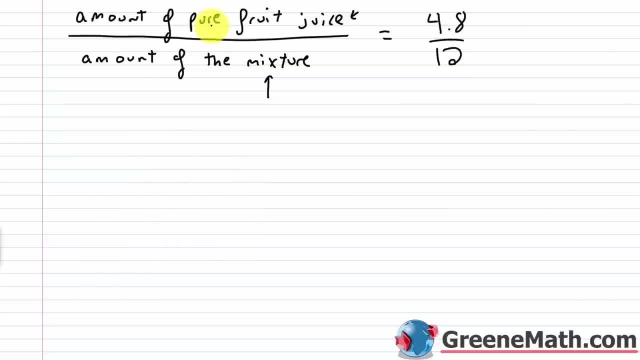 So again, what I figured out was the amount of pure fruit juice. I have 4.8 liters. And I know the amount of the mixture. That's 12 liters. 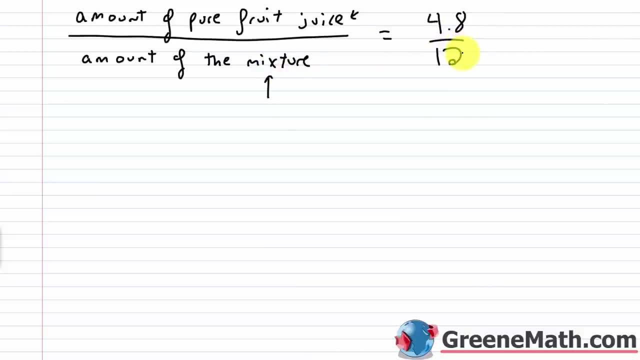 If I divide one by the other, I'm going to get as a decimal 0.4. 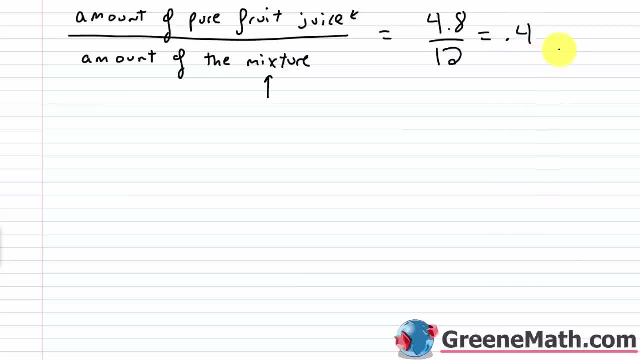 So as a percentage, I just move this guy over two places to the right, and I have 40%. 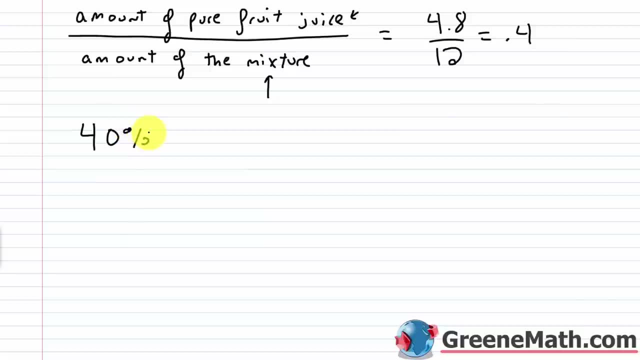 So that means that my mixture is going to be 40% fruit juice. So I can come back up here. What is the percentage of fruit juice in the mixture? 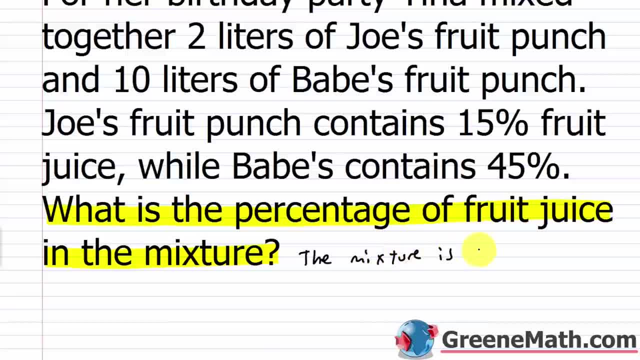 The mixture is 40% fruit juice. 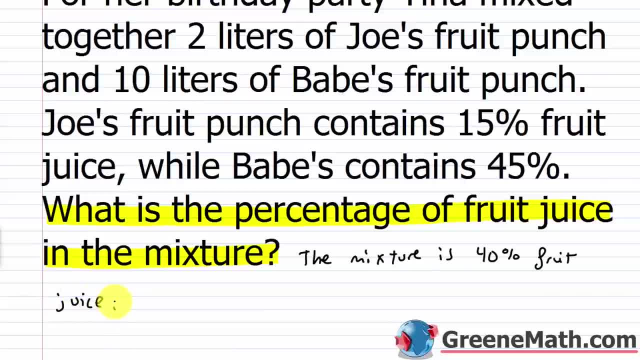 And it's kind of easy to check that. I mean, this is a very simple one. 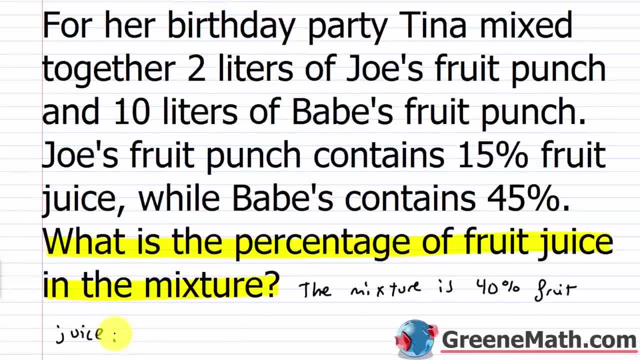 So Tina mixed 2 liters of Joe's Fruit Punch and 10 liters of Babes Fruit Punch. 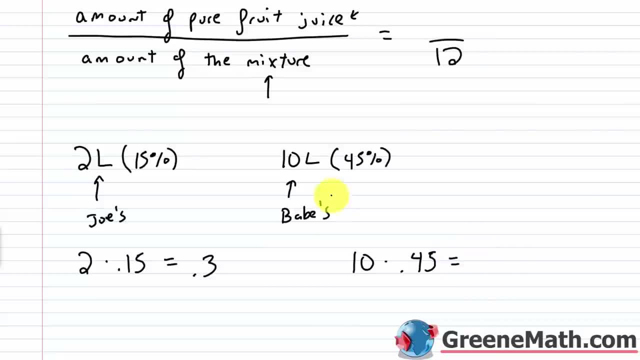 that's going to give me the amount of pure fruit juice that I'm throwing in from Babes fruit punch. So this is going to be 4.5.. So if I sum these two amounts together the amount of pure fruit juice that I'm putting in from Joe's plus the amount of pure fruit juice that I'm putting. 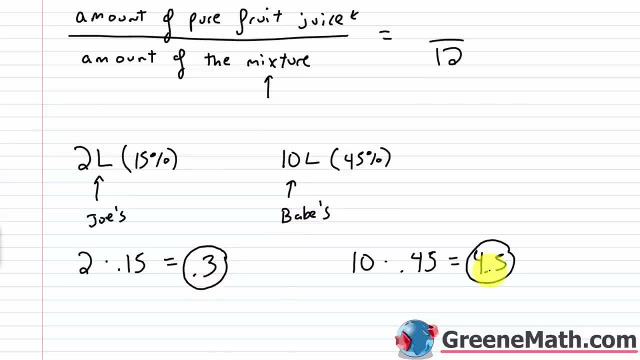 in from Babes, I'd get 4.8, right, 0.3 plus 4.5 is 4.8.. So essentially I have 4.8 divided by 12.. So let's erase this real quick. We'll do our calculation. So again what I figured. 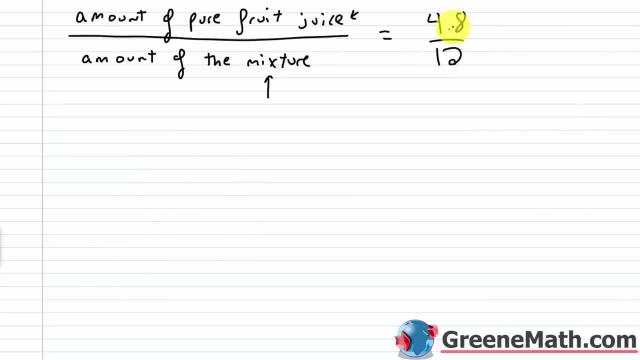 out was the amount of pure fruit juice. I have 4.8 liters and I know the amount of the mixture. that's 12 liters. If I divide one by the other, I'm going to get 5.8 liters. So this is the amount of pure. 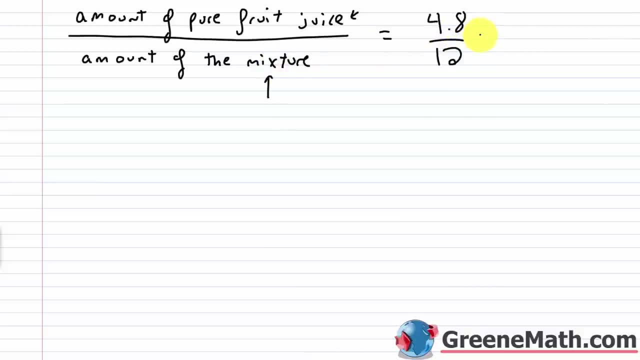 fruit juice that I'm putting in from Joe's, plus the amount of pure fruit juice that I'm putting in from Babes, I'm going to get, as a decimal, 0.4.. So as a percentage, I just moved this guy over two. 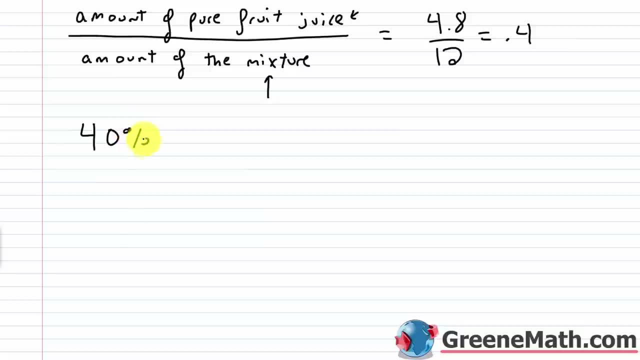 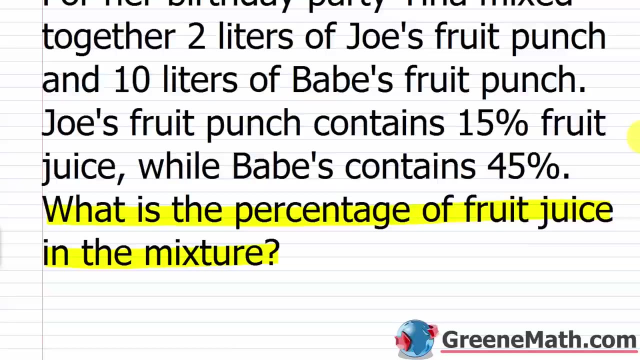 places to the right and I have 40%. So that means that my mixture is going to be 40% fruit juice. So I can come back up here. What is the percentage of fruit juice in the mixture? The mixture is 40% fruit juice. 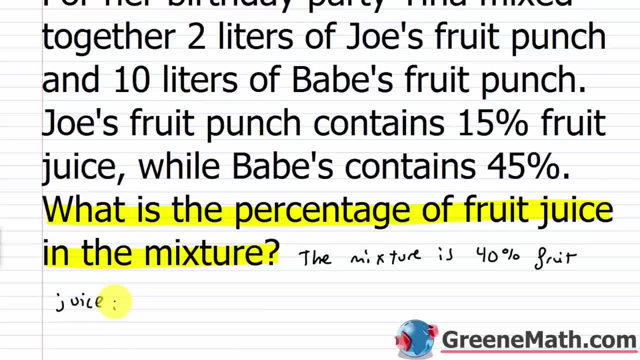 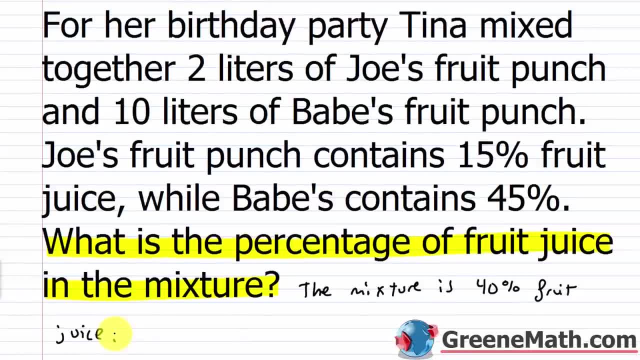 And it's kind of easy to check that. I mean, this is a very simple one. So Tina mixed two liters of Joe's fruit punch and 10 liters of Babes fruit punch. Again, two plus 10 is 12.. So that's the total amount of the mixture. Now, Joe's fruit punch contains 15% fruit juice. 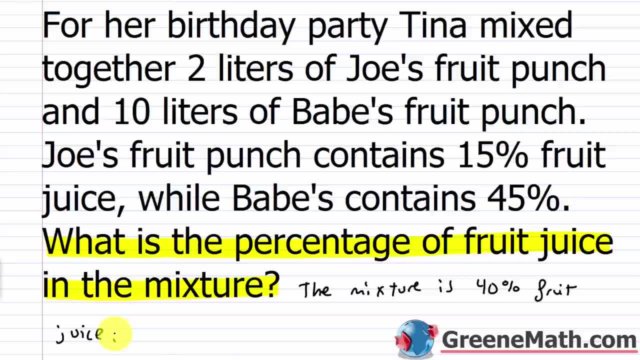 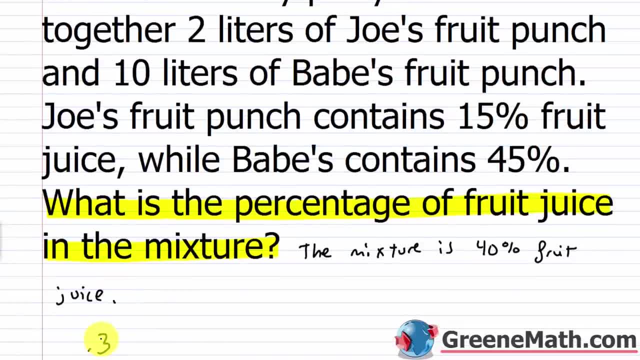 So if I take two liters, or just the number two, and I multiply it by 15% or in decimal form, 0.15,, that means that I have 0.3 liters of pure fruit juice. That's the amount of pure fruit juice. 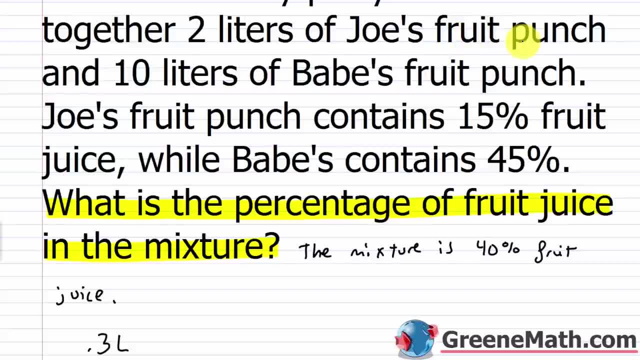 That's coming from Joe's fruit punch, Now from Babes fruit punch, I've got 10 liters and it's 45% fruit juice. So I'm getting 4.5 liters of pure fruit juice there. Combine these two together through addition And what I'd have is I'd have 4.8 liters of pure fruit. Again, 2 plus 10 is 12. 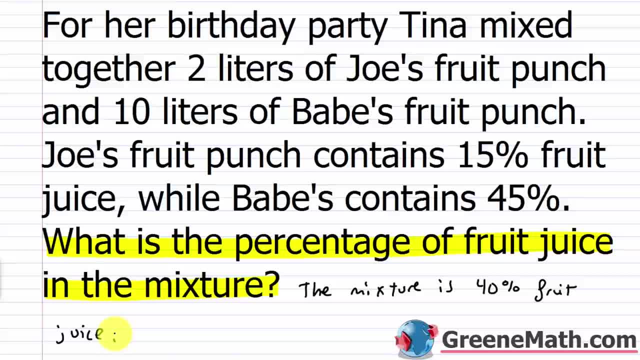 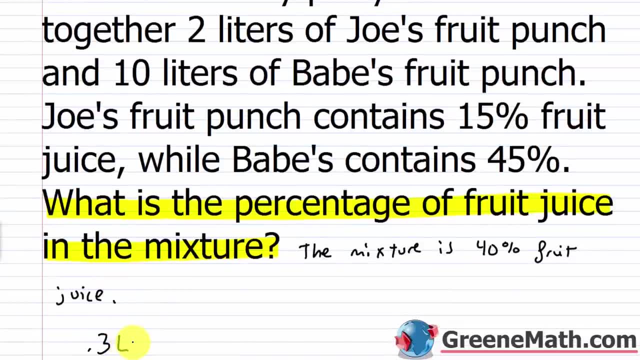 So that's the total amount of the mixture. Now Joe's Fruit Punch contains 15% fruit juice. So if I take 2 liters, or just the number 2, and I multiply it by 15%, it will form 0.15. That means that I have 0.3 liters of pure fruit juice that's coming from Joe's Fruit Punch. 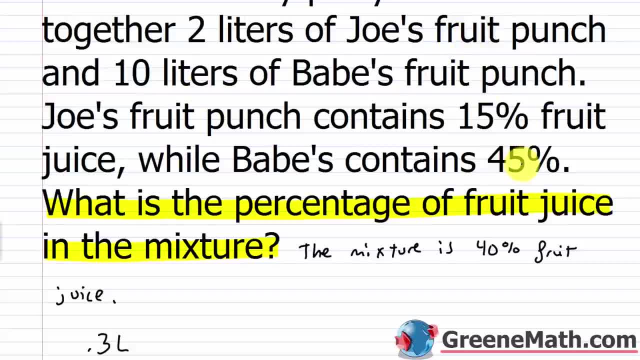 Now from Babes Fruit Punch, I've got 10 liters, and it's 45% fruit juice. So I'm getting 4.5 liters of pure fruit juice there. 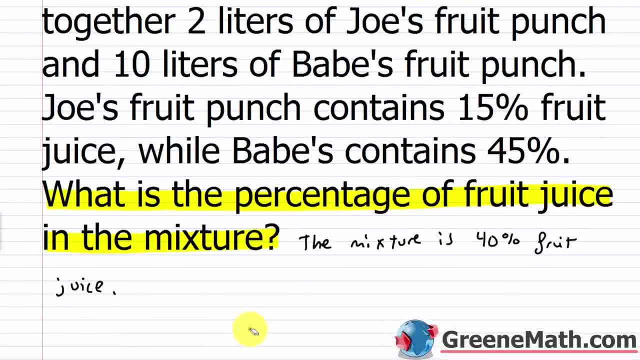 Combine these two together through addition, and what I'd have is I'd have 4.8 liters of pure fruit juice, 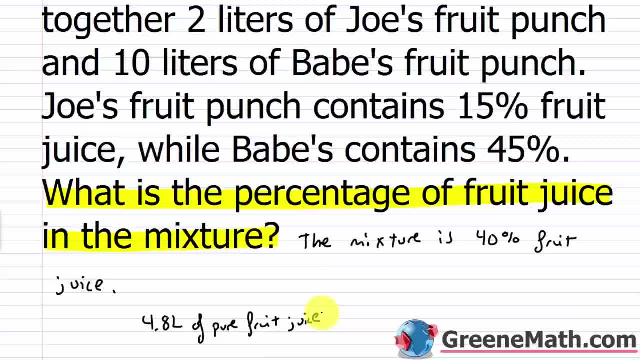 in the mixture that is a total of 12 liters. 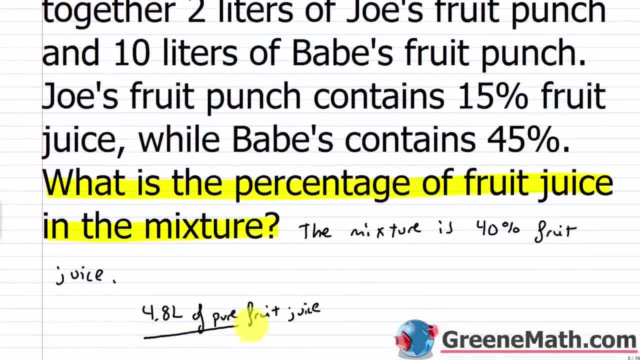 So all you'd have to do is take 4.8 and divide it by 12, which is the total number of liters in the mixture. 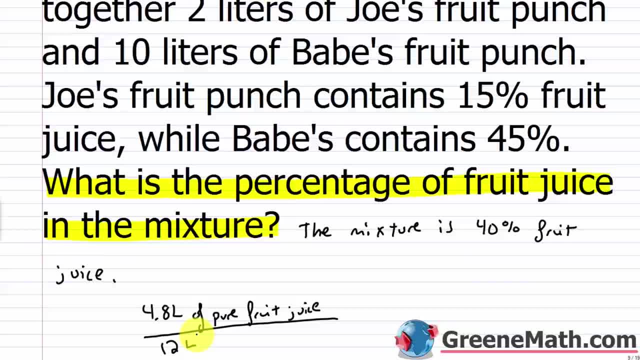 That gives me 0.4, and so as a percentage, that's 40. So 40% of this mixture is going to be pure fruit juice. Alright, so let's take a look at a harder one now. 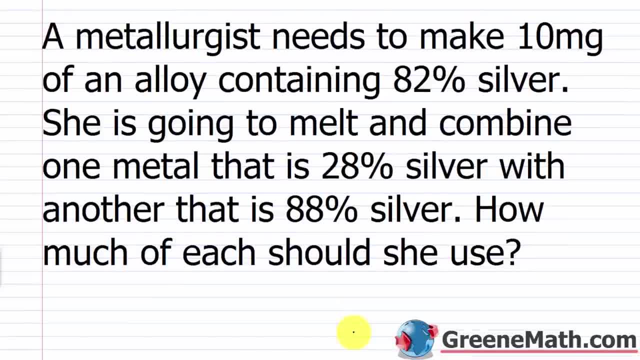 One that's going to involve the use of variables to solve. 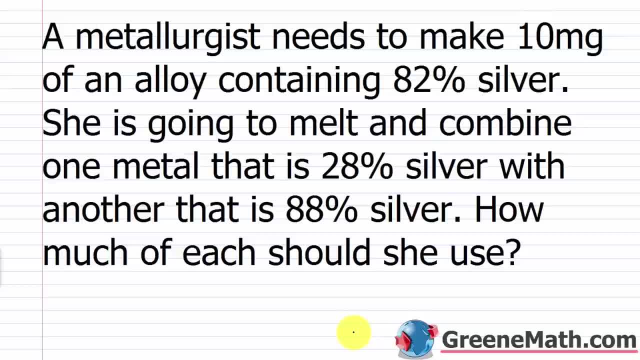 So a metallurgist, needs to make 10 milligrams of an alloy 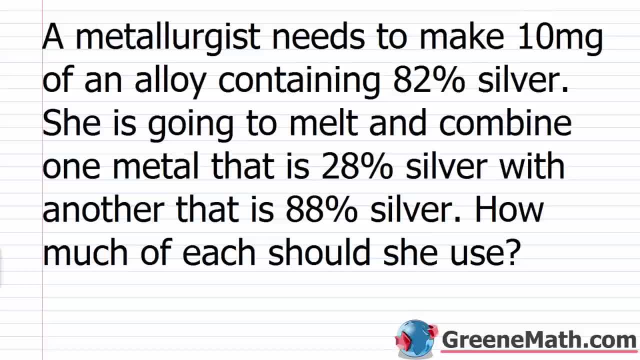 containing 82% silver. So let's stop for a second. 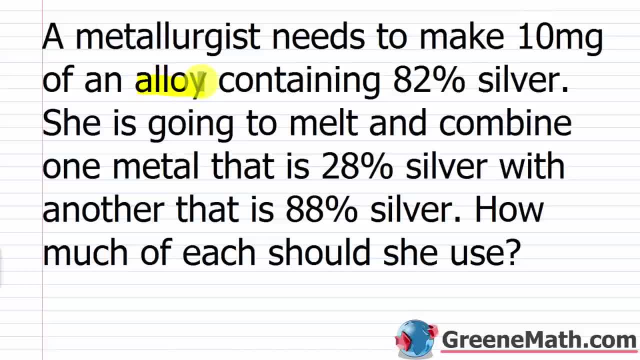 Some of you don't know what an alloy is. So an alloy 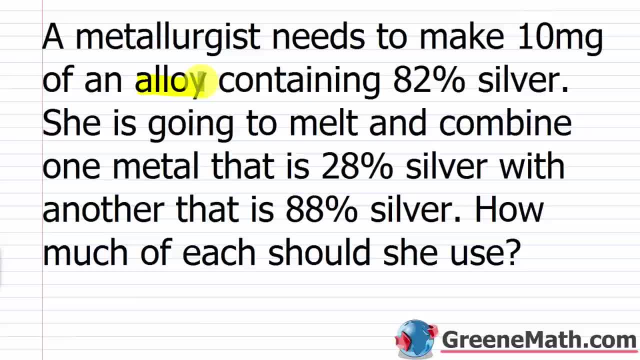 is a metal that's made by combining two or more metallic elements. 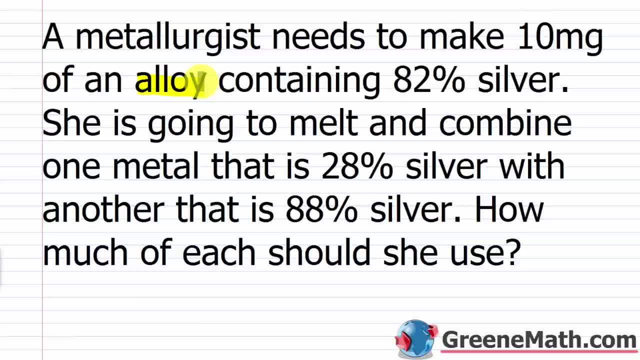 Alright, so then she is going to melt and combine one metal that is 28% silver, let me highlight that, 28% silver, with another that is 88% silver. 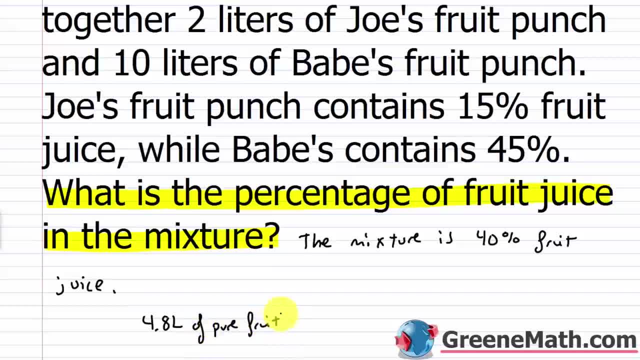 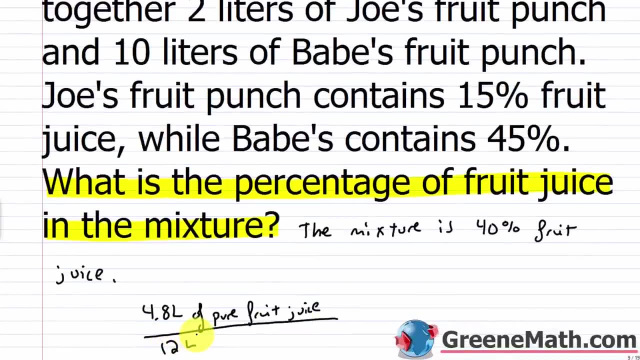 juice in the mixture. That is a total of 12 liters. So all you'd have to do is take 4.8 and divide it by 12, which is the total number of liters in the mixture. That gives me 0.4, and so as a percentage, that's 40. So 40% of this. 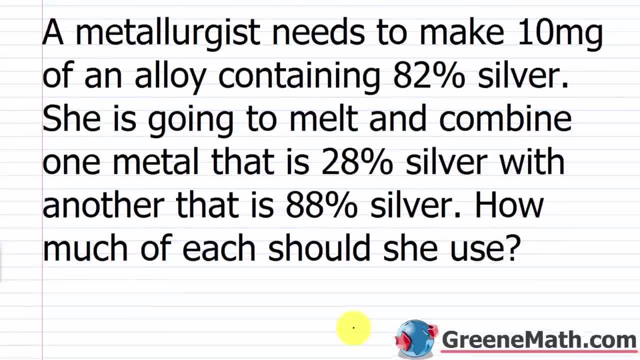 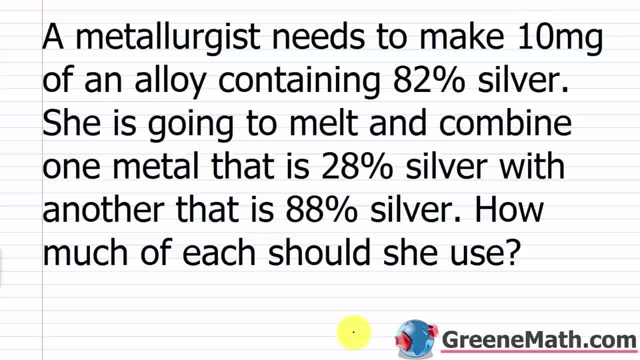 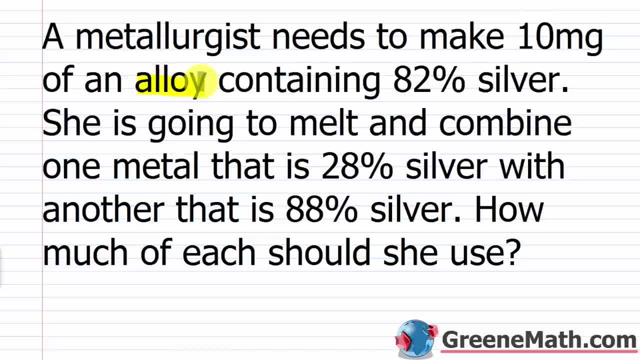 stop for a second. Some of you don't know what an alloy is. So an alloy is a metal that's made by combining two or more metallic elements. Alright, so then she is going to melt and combine one metal that is 28% silver. Let me highlight that: 28% silver with another. 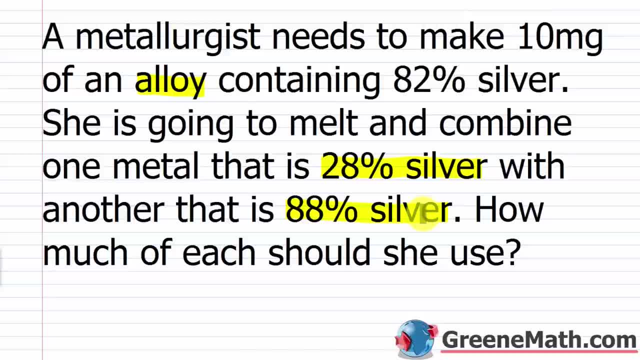 that is 88% silver. How much of each should she use? So here's our question: How much of each should she use, Meaning how much in terms of milligrams should she use of the one metal that's 28% silver? How much in terms of milligrams should she use of the other? 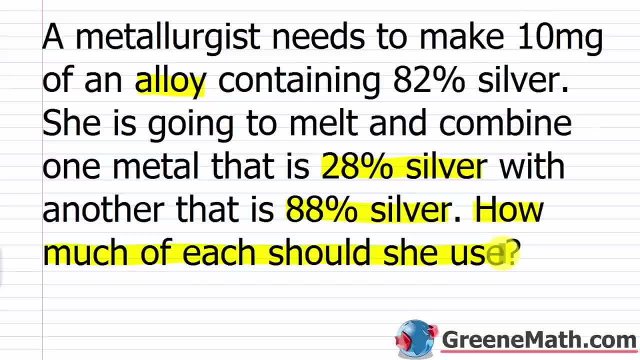 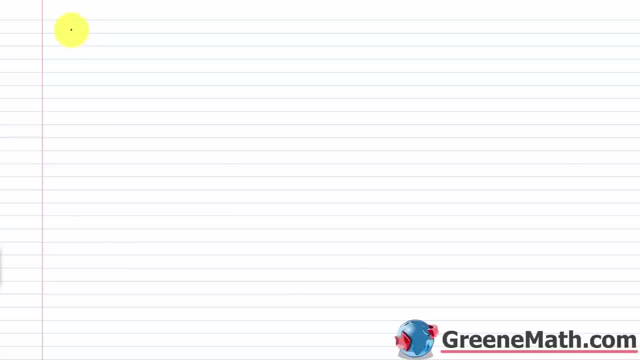 metal that is 88% silver. So when we move to our next step and we want to assign a variable to represent the unknown, we have those two unknowns, So let's let X equal one of those. So let's let it equal. 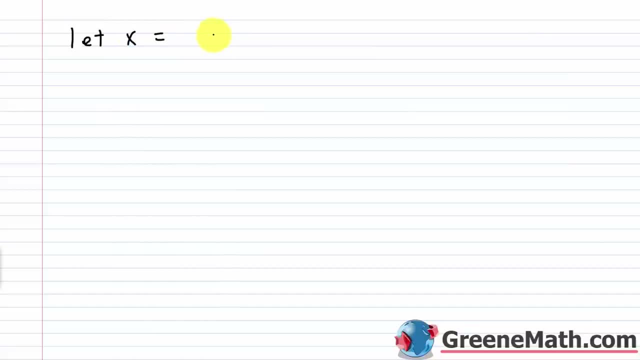 Let's let X equal the amount of metal in milligrams, that is 28% silver. Okay, So the amount of metal in milligrams, that is 28% silver. Now to express the other unknown in terms of X. you kind of have to read through the problem. This is a little tricky. the first: 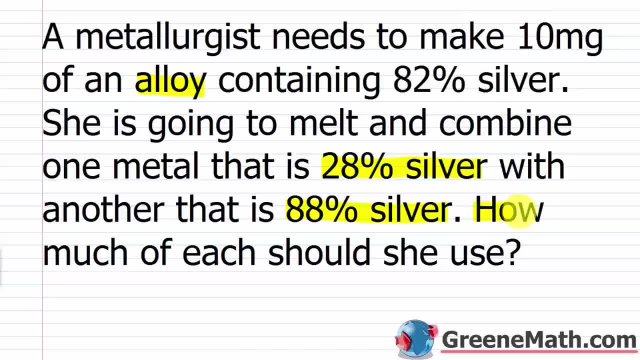 How much of each should she use? So here's our question. How much of each should she use? Meaning, how much, in terms of milligrams, should she use of the one metal that's 28% silver? How much, in terms of milligrams, should she use of the other metal that is 88% silver? 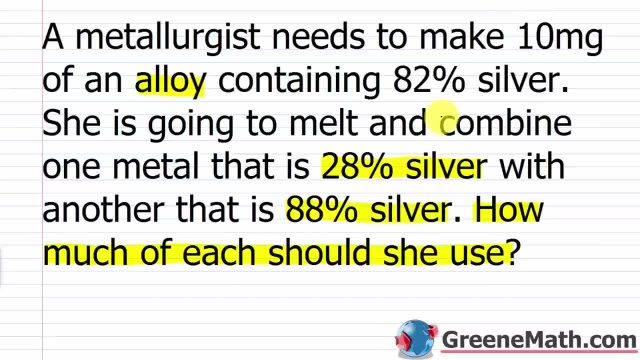 So when we move to our next step and we want to assign a variable to represent the unknown, we have those two unknowns. 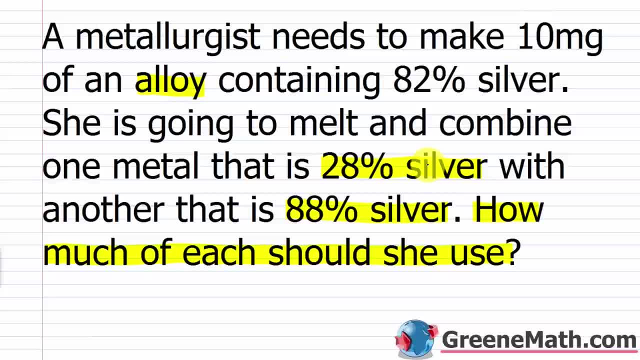 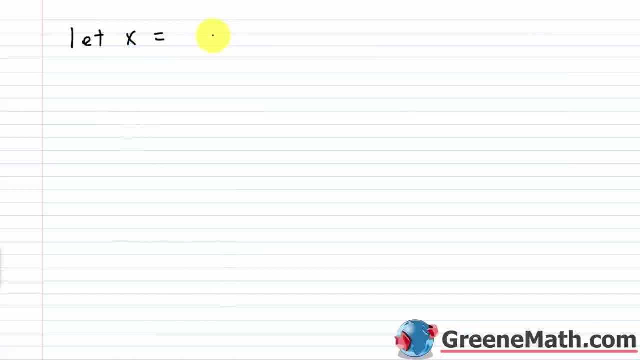 So let's let x equal one of those. So let's let x equal one of those. So let's let it equal, let's let x equal let's let x equal the amount the amount of metal of metal in milligrams in milligrams 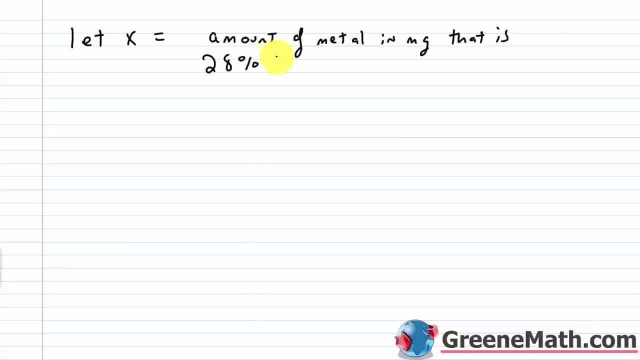 that is 28% that is 28% silver. Okay. 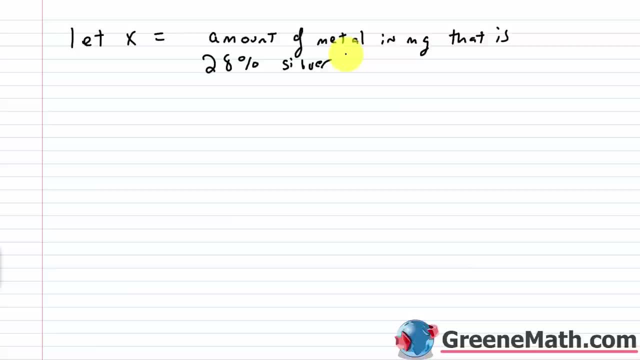 So the amount of metal in milligrams that is 28% silver. 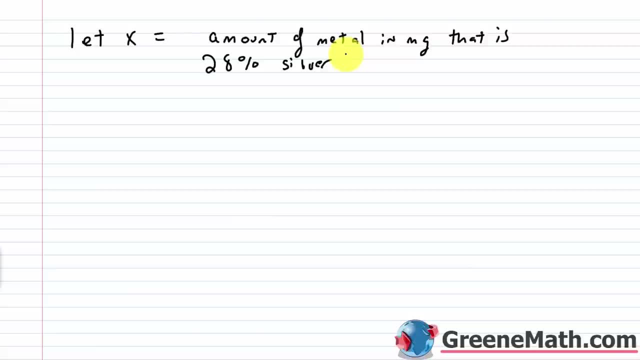 To express the other unknown in terms of x, you kind of have to read through the problem. 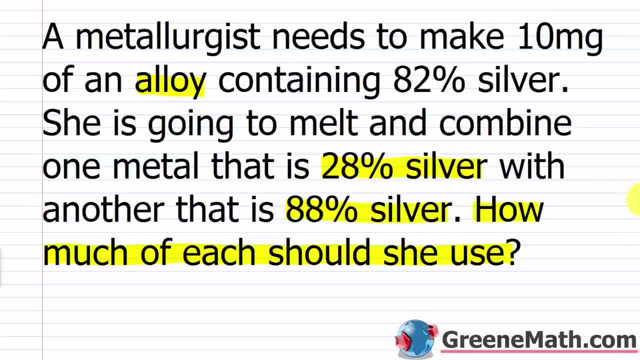 This is a little tricky the first time, so I have to kind of walk you through it. Here's the information that you might have missed. 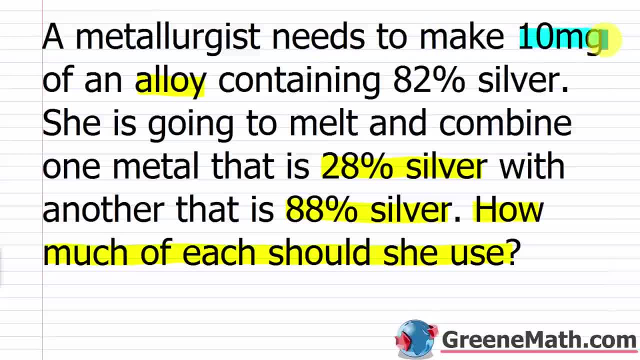 A metallurgist needs to make 10 milligrams of an alloy containing 82% silver. This is the first key. 10 milligrams. 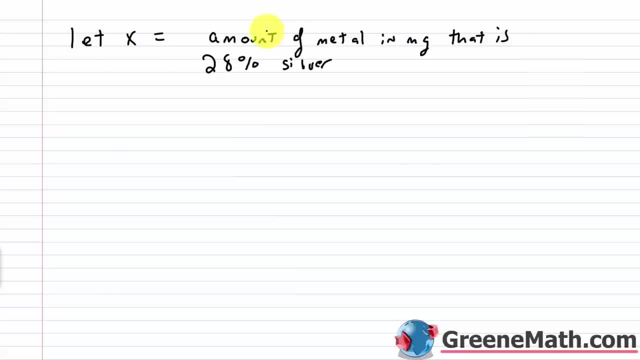 So we know that x is the amount of metal in milligrams that is 28% silver. So whatever x is, if I add the other amount to it, the sum should be 10, in terms of milligrams. x milligrams plus some other amount of milligrams should equal 10 milligrams. 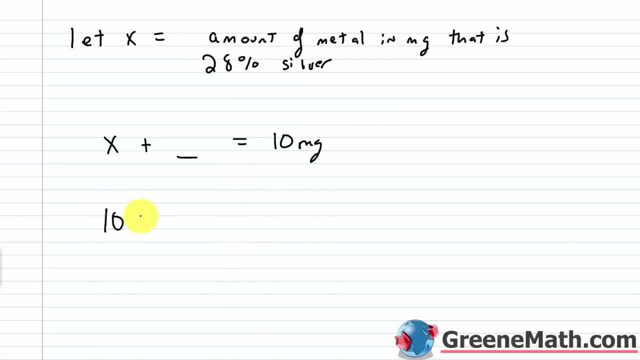 So now I can kind of work backwards and say 10 is equal to x plus this amount here can only be 10 minus whatever x is. And I know that's a little tricky at first, but 10 minus whatever this is, let's say x was 4 for example. 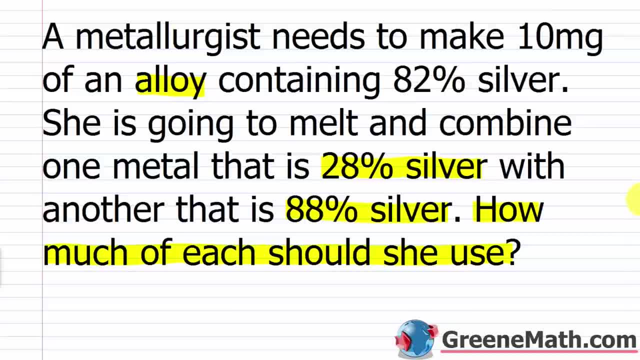 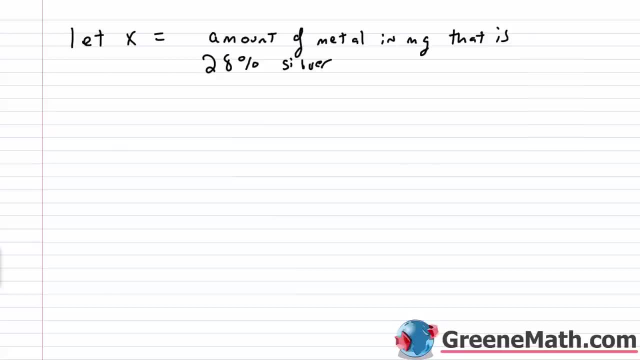 time, so I have to kind of walk you through it. Here's the information that you might have missed: A metallurgist needs to make 10 milligrams of an alloy containing 82% silver. This is the first key, 10 milligrams. So we know that X is the amount of metal in milligrams. 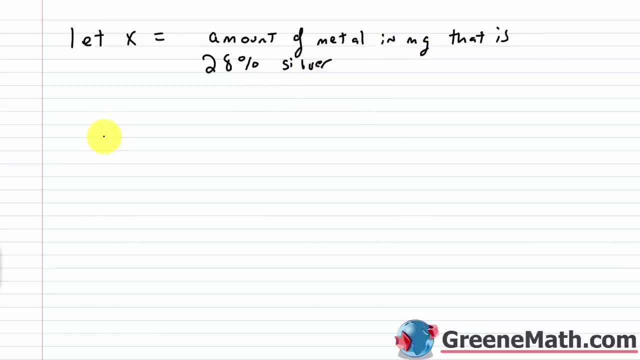 that is 28% silver. So, whatever X is, if I add the other amount to it, the sum should be 10,. right. in terms of milligrams, right, It should be 10 milligrams. X milligrams plus some other amount of milligrams should equal. 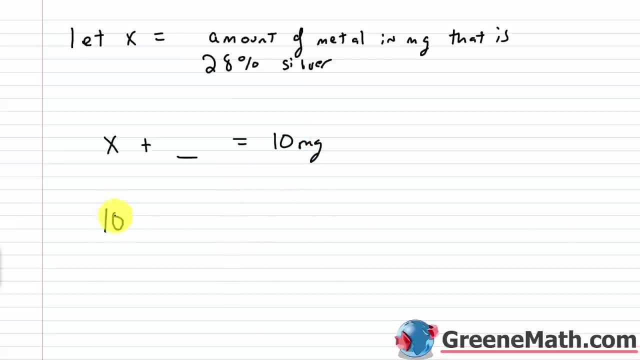 10 milligrams. So now I can kind of work backwards and say: okay, well, 10 is equal to X plus This amount. here can only be 10 minus whatever X is- And I know that's a little tricky at first- but 10 minus whatever this is. 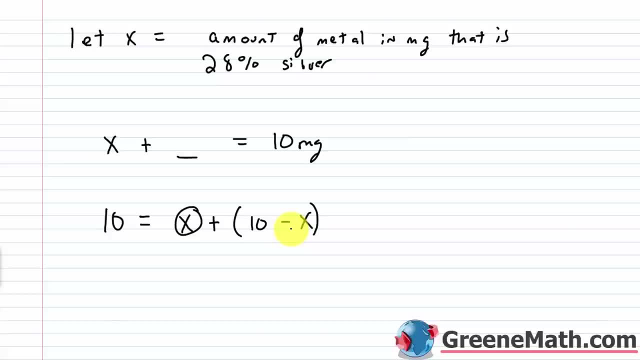 Let's say X was four, for example. I'm not saying that's the answer, but let's just say X was four. So if this was four, 10 minus four would be six. So four plus six would be 10.. In other words, whatever X is, 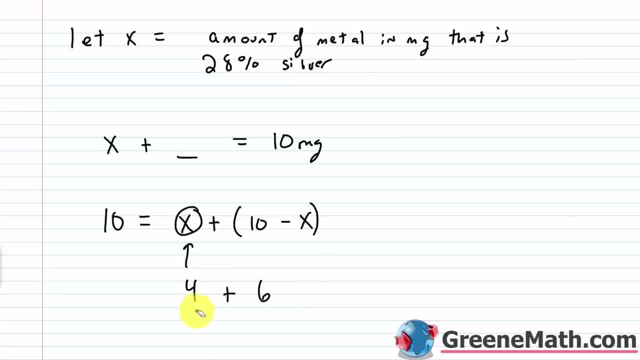 the other amount, when added to that, has to sum to 10.. So that's why this would work out. So if, let's say, X was eight, then this amount would have to end up being two, right, Because these two amounts have to sum to 10.. So that's where you're going to get this formula from. 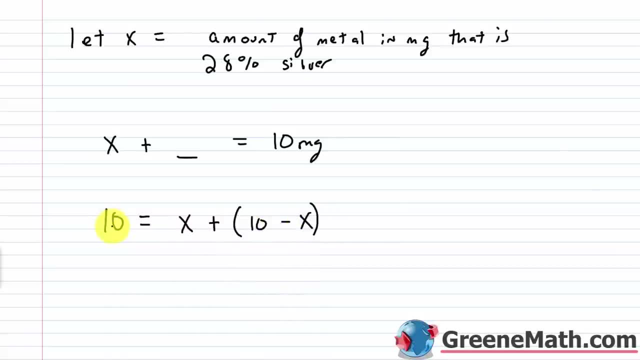 So X plus 10 minus X is going to equal 10.. Now that gives us our relationship for the other metal. So we could say then 10 minus X is going to be the amount of metal in milligrams, that is, 88% silver. 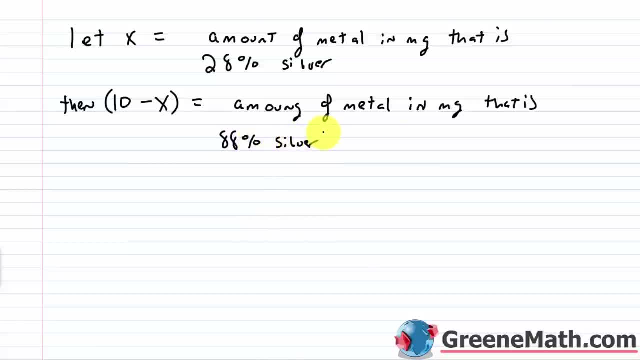 Okay, Okay, Okay, Okay. And again, I know the first time. you see that it's a little confusing, but as you work through these problems, that's going to become something you look for all the time. All right, So now we want to set up an equation So some of you might immediately make the 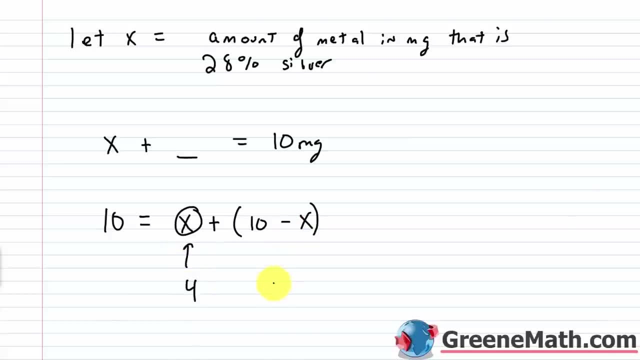 I'm not saying that's the answer, but let's just say x was 4. So if this was 4, 10 minus 4 would be 6. So 4 plus 6 would be 10. In other words, whatever x is, the other amount when added to that has to sum to 10. So that's why this would work out. 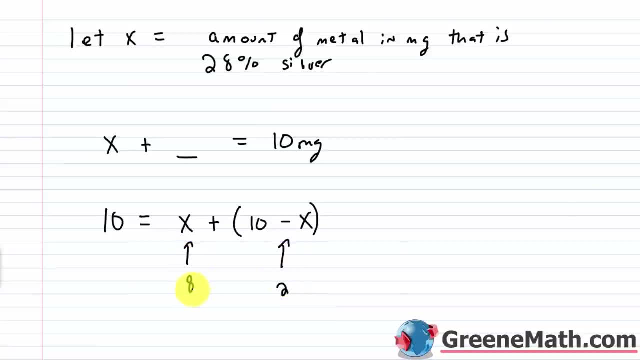 So if let's say x was 8, then this amount would have to end up being 2. 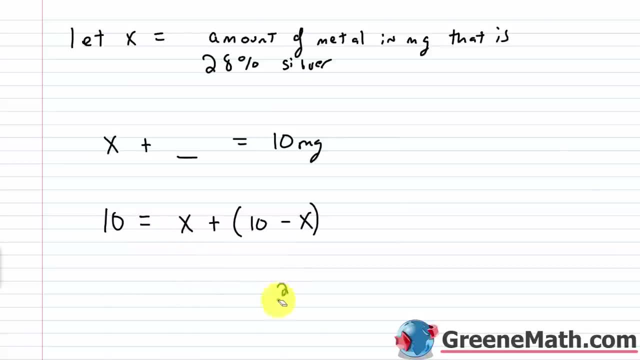 Because these two amounts have to sum to 10. So that's where you're going to get this formula from. 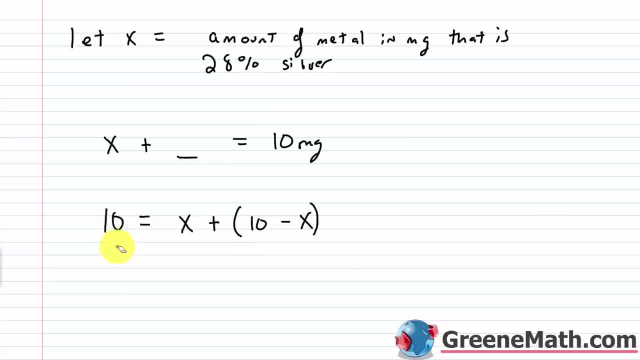 10 minus x is going to equal 10. Now, that gives us our 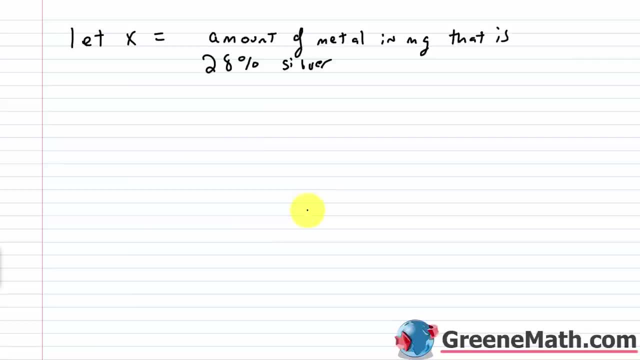 relationship for the other metal. So we can say then 10 minus x is going to be the amount 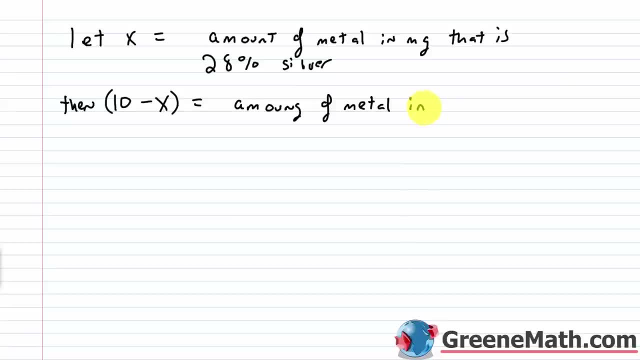 of metal in milligrams that is 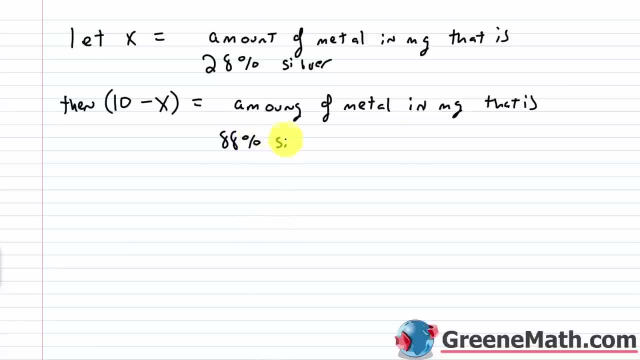 88% silver. And again, I know the first time you see that it's a little confusing, but as you work through these problems, that's going to become something you look for all the time. 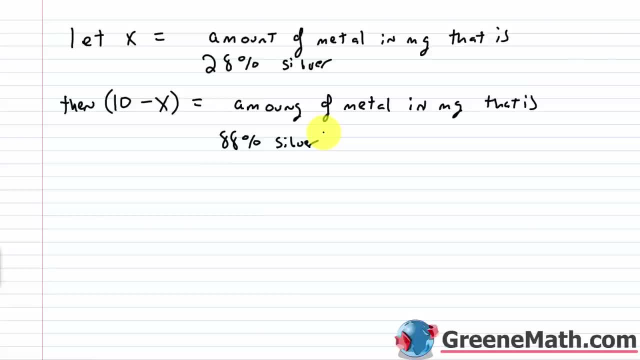 Alright, so now we want to set up an equation. So some of you might immediately make the mistake and say, okay, well I know the weights. So my equation is x plus 10 minus x equals 10. Okay, let's go through and solve this. 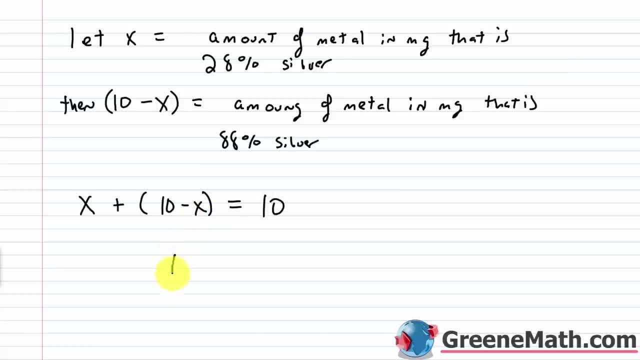 x minus x is 0, and then I have 10 equals 10. 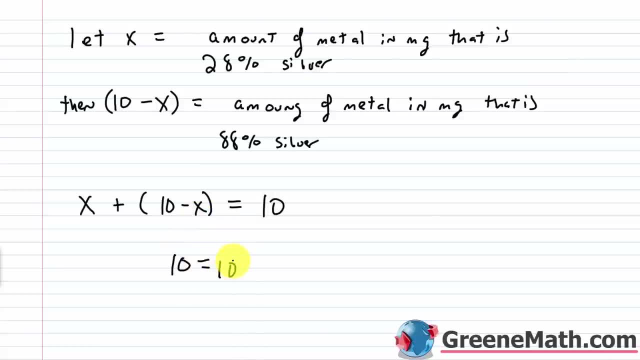 And you might go, okay, what happened? What's wrong here? 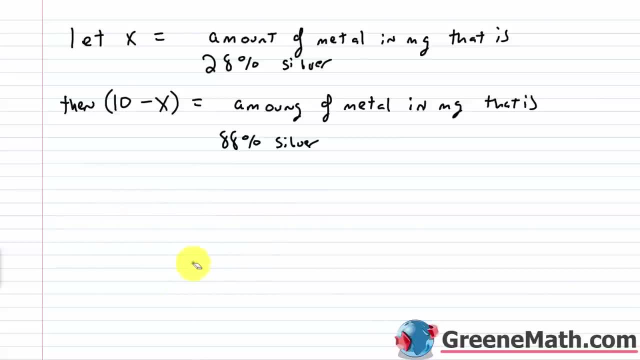 Well, you don't have enough information. What you need here is to relate the fact that, okay, you have a certain weight for x, but 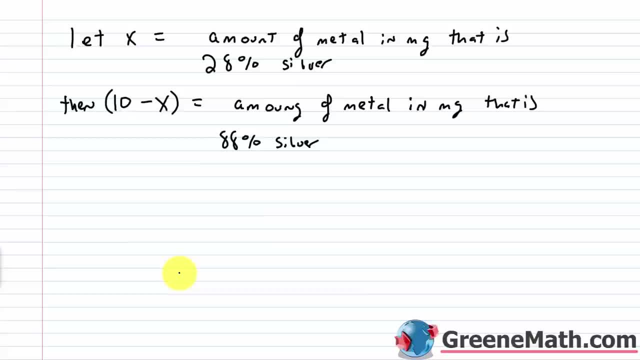 that weight is a certain percentage of silver. 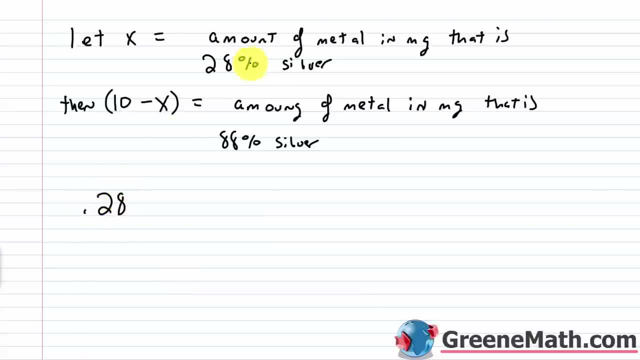 So if 0.28 right, 28% as a decimal is 0.28, times x is used to represent the amount of metal in milligrams of pure silver. 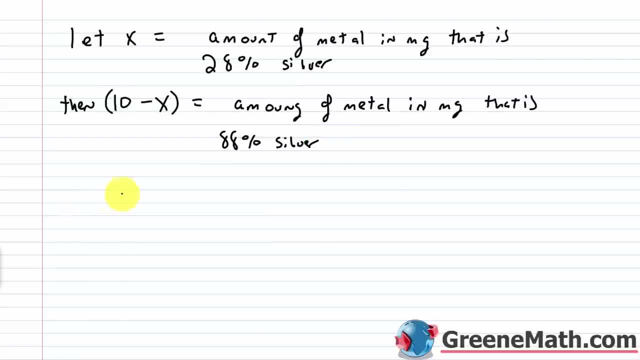 mistake and say: okay, well, I know the weights. So my equation is: X plus 10 minus X equals 10.. I might say: okay, let's go through and solve this. X minus X is zero, and then I have 10 equals 10.. And you might go. okay, what happened? 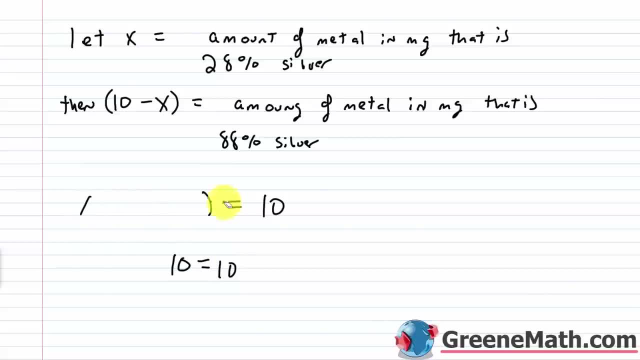 what's wrong here? well, you don't have enough information. what you need here is to relate the fact that, okay, you have a certain weight for X, but that weight is a certain percentage of silver. so if 0.28- right, twenty eight percent as a decimal- is 0.28 times X is used to represent the amount in milligrams of. 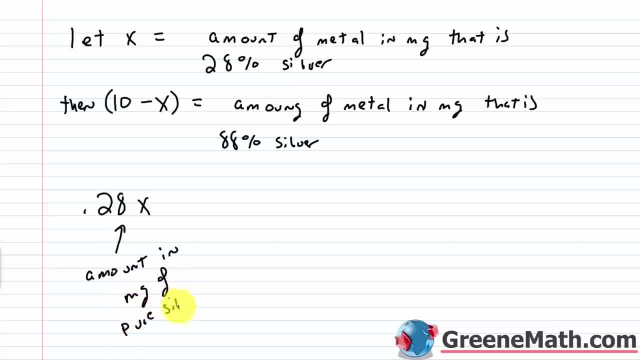 pure silver. then we add this to now we have the amount of metal in milligrams. that's 88% silver, so 0.88, which is 88% as a decimal times. this- remember to use this parentheses here- 10 minus X. very important, okay, you can't just put it next to the 10, that won't work. this is the same. 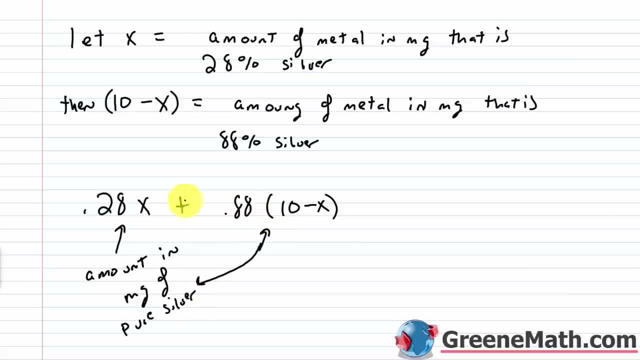 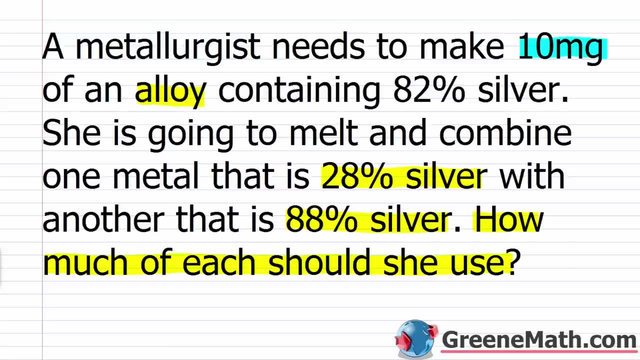 thing. it's the amount in milligrams of pure silver. so these two amounts have to be equal to what it told us in the problem. and in the problem it says that the metallurgist needs to make 10 milligrams of an alloy containing 82%. 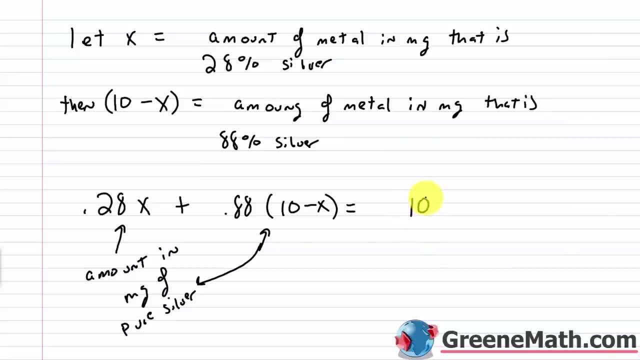 silver. so 10 is the total weight and the percentage is 82%, so 0.82. and so now we have an equation, now we have something we can solve. so amount in milligrams of pure silver is equal to the amount in milligrams of pure silver. 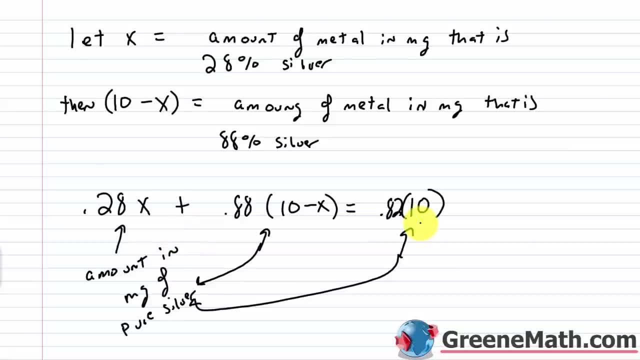 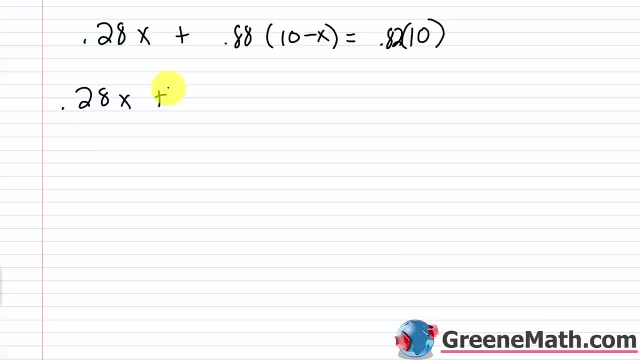 one side is going to be equal to the other and we have something we can work with. let's go ahead and solve the equation now, so we'll have 0.28 X plus 0.88 times 10. I'm just gonna move this one place to the right, so that would be. 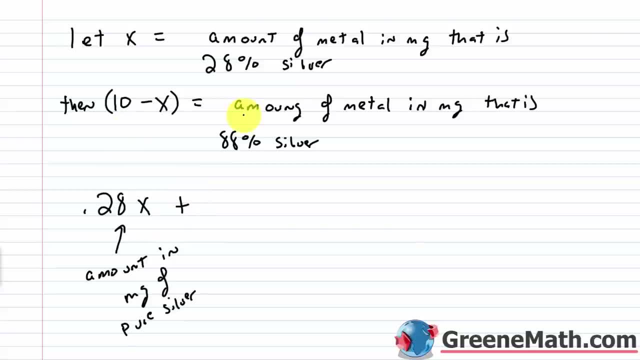 Then we add this to, now we have the amount of metal in milligrams that's 88% silver, so 0.88, which is 88% as a decimal, times this, remember to use this parentheses here, 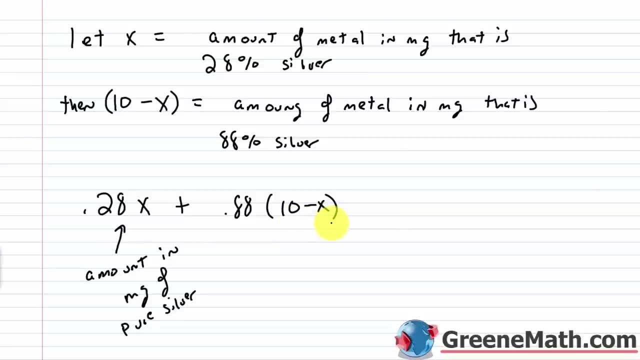 10 minus x, very important. You can't just put it next to the 10, that won't work. 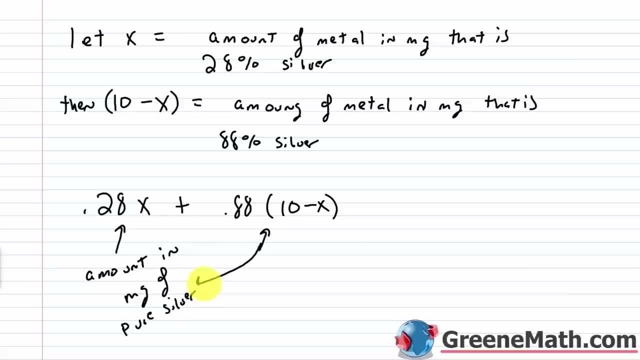 This is the same thing, it's the amount in milligrams of pure silver. 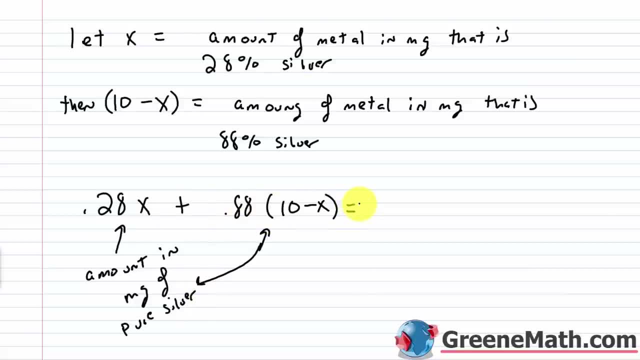 So these two amounts have to be equal to what it told us in the problem. And in the problem it says that the metallurgist needs to make 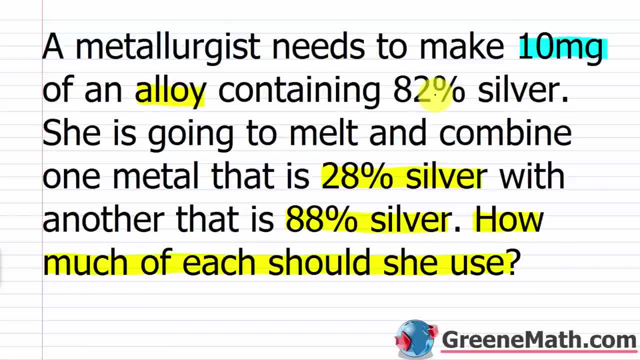 10 milligrams of an alloy containing 82% silver. 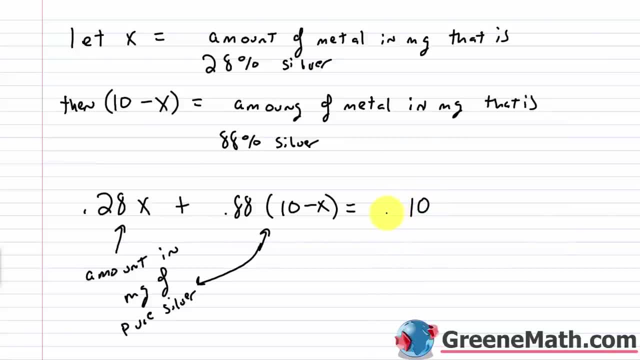 So 10 is the total weight, and the percentage is 82%, so 0.82. 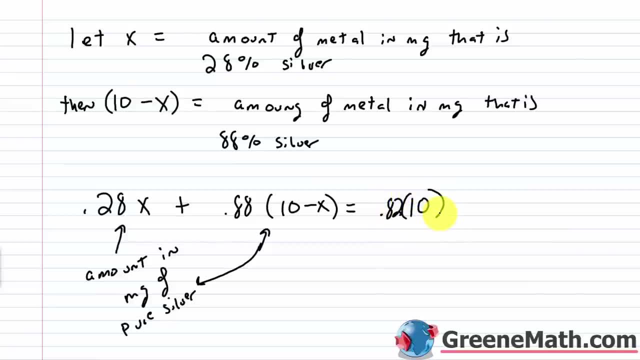 And so now we have an equation. Now we have something we can solve. So amount in milligrams of pure silver is equal to the amount in milligrams of pure silver. One side is going to be equal to the other, and we have something we can work with. 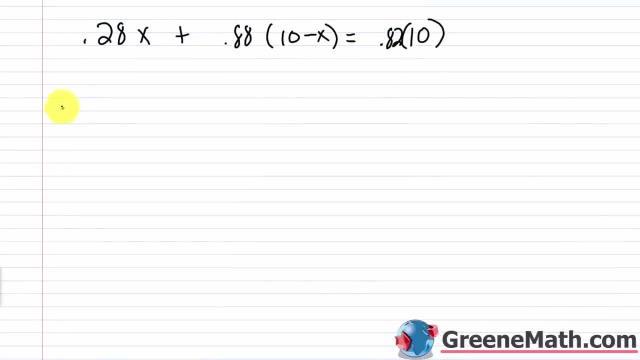 Let's go ahead and solve the equation now. So we'll have 0.28x plus 0.88 times 10. I'm just going to move this one place to the right, so that would be 8.8. Then minus 0.88 times x is 0.88x. Then equals 0.82 times 10 is 8.2. 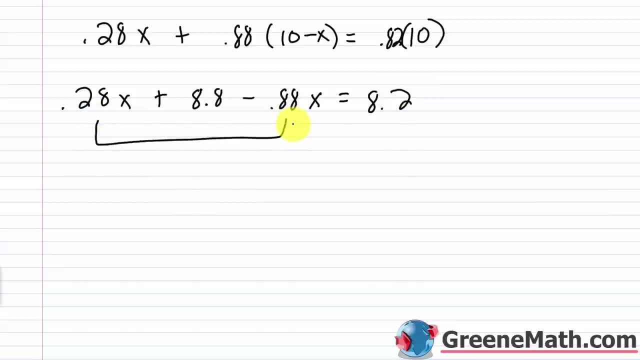 So if we combine like terms here, 0.28x minus 0.88x is going to give me negative 0.6x. Then plus 8.8 equals 8.2. I'm going to subtract 8.8 away from each side of the equation. 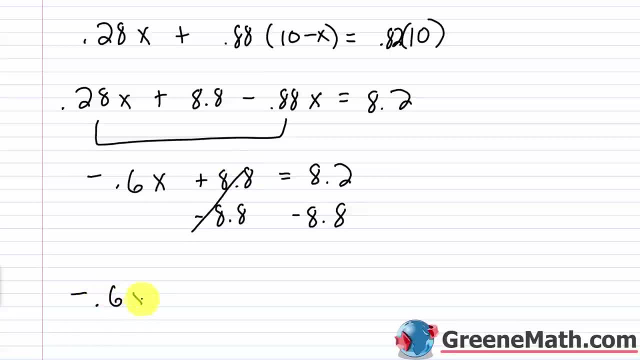 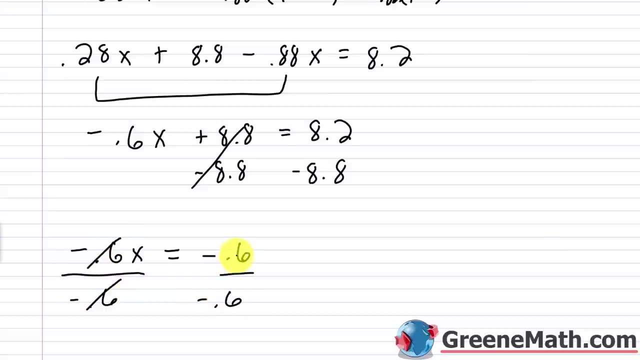 That's gone. I'm going to have negative 0.6x is equal to 8.2 minus 8.8 is going to be negative 0.6. Divide both sides of the equation by negative 0.6, the coefficient of x. That's going to cancel with that, and this is going to cancel out also and become 1. 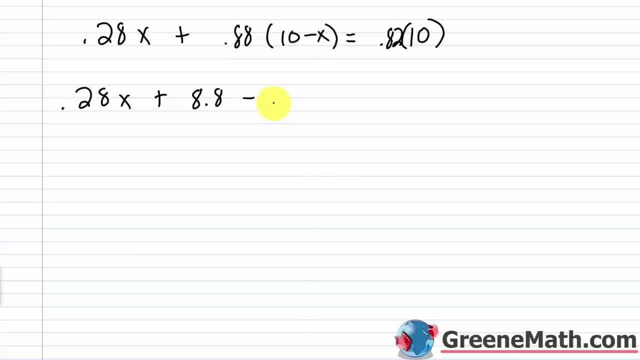 eight point eight and minus point eight. eight times X is point eight. eight X is and equals 0.82 times 10 is 8.2.. So if we combine like terms here, 0.28x minus 0.88x is going to give me negative 0.6x. Then plus 8.8 equals 8.2.. I'm going to subtract 8.8 away. 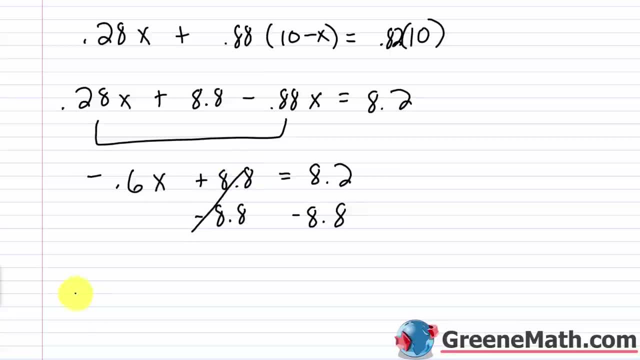 from each side of the equation. That's gone, I'm going to have negative. 0.6x is equal to 8.2 minus 8.8 is going to be negative 0.6.. Divide both sides of the equation by negative 0.6, the coefficient. 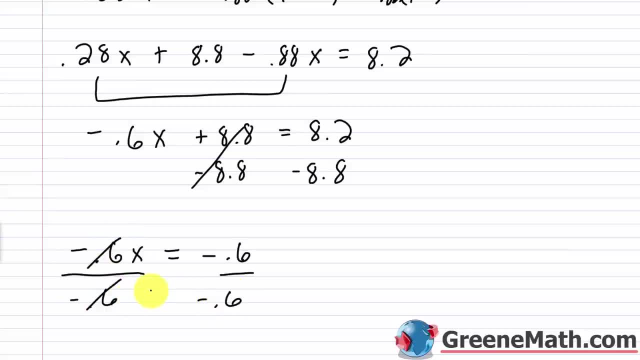 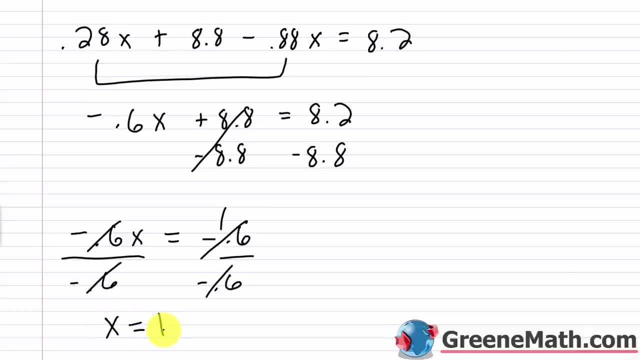 of x, That's going to cancel with that, And this is going to cancel out also and become 1.. So we have x equals 1.. All right, so let's make sense of this. Remember that x is the amount of metal. 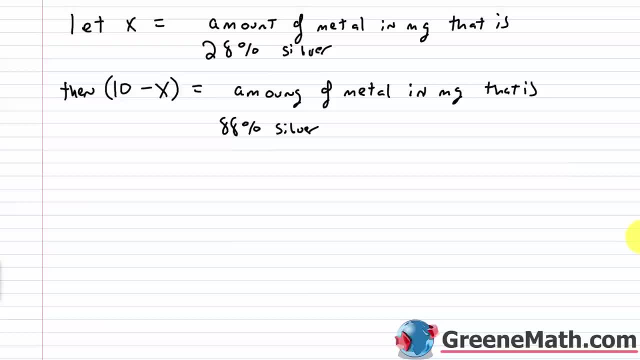 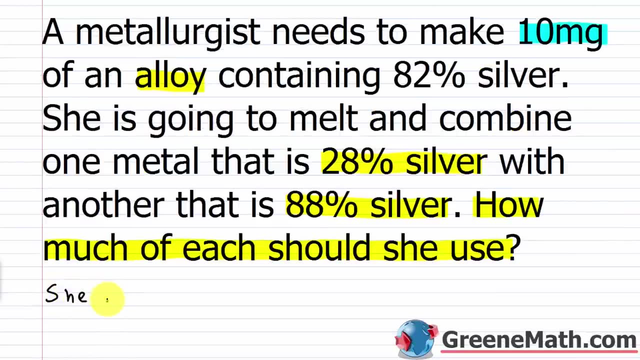 in milligrams, that is 28% silver. So that we said was 1, because x was equal to 1 when we solved our equation. So we're going to say that she needs 1 milligram of the metal- that is 28% silver, And then, along with 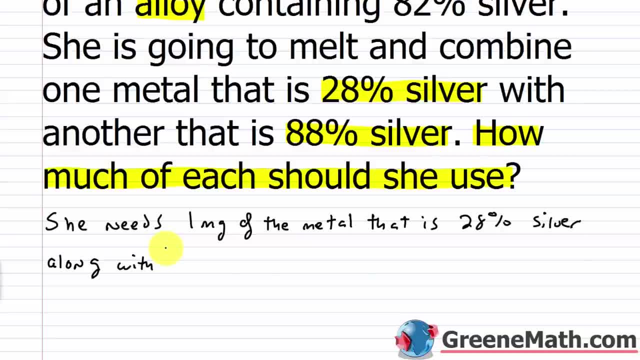 10,, which is the total weight of this thing, minus 1, which is the weight of the metal, that is, 28% silver, so 9.. So, along with 9 milligrams- remember we set that up as 10 minus x 10 minus. 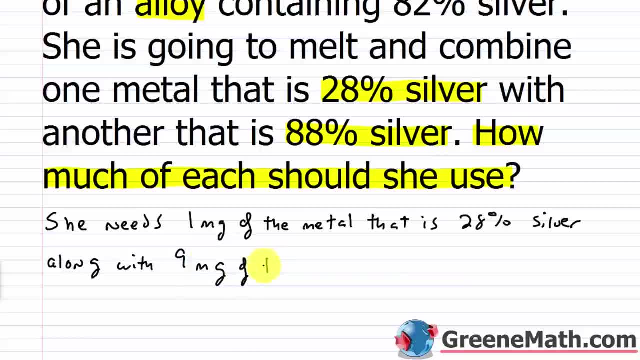 1 would be 9.. So, along with 9 milligrams of the metal, that is 88% silver. So that's what she's going to use to make this. She's going to use this alloy, that is 10 milligrams and 82% silver. So check everything out If you go. 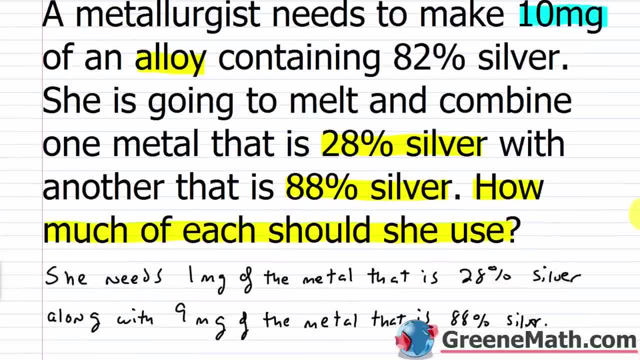 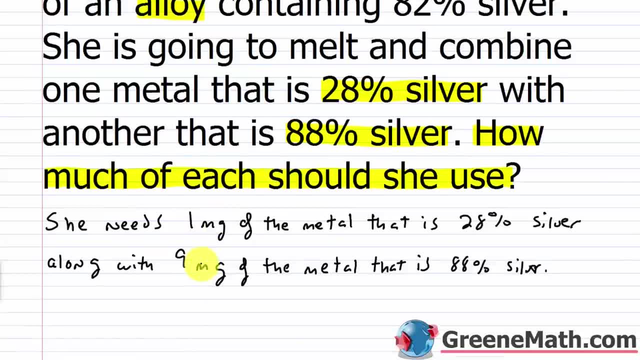 back up again. a metallurgist needs to make 10 milligrams of an alloy containing 82% silver. So we know that 1 milligram plus 9 milligrams is 10 milligrams. So that part checks out, We just. 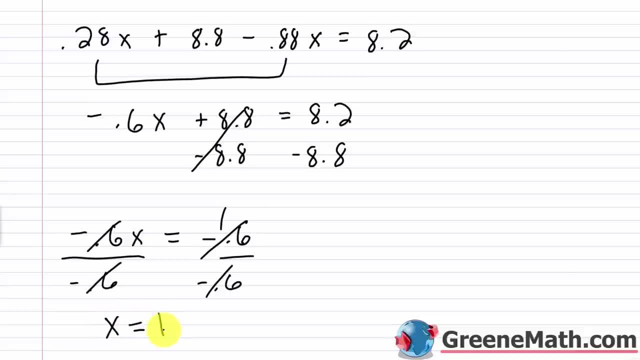 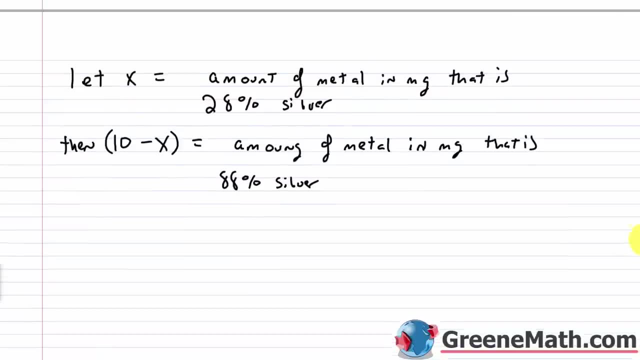 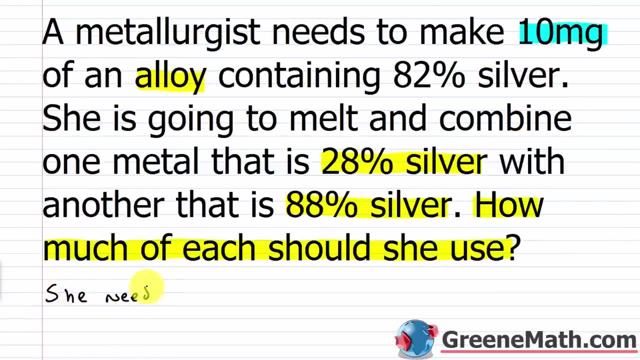 So we have x equals 1. Alright, so let's make sense of this. Remember that x is the amount of metal in milligrams that is 28% silver. So that we said was 1. Because x was equal to 1 when we solved our equation. So we're going to say that she needs 1 milligram of the metal 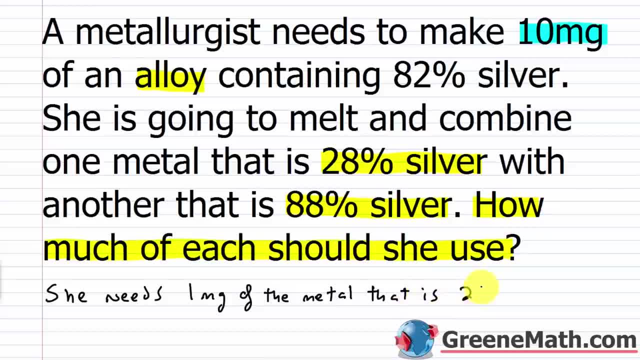 that is 28% silver. 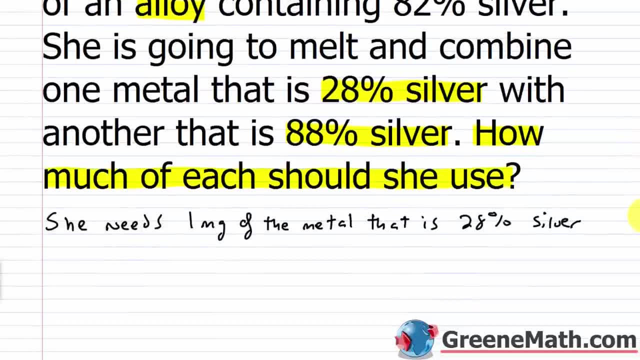 And then along with along with 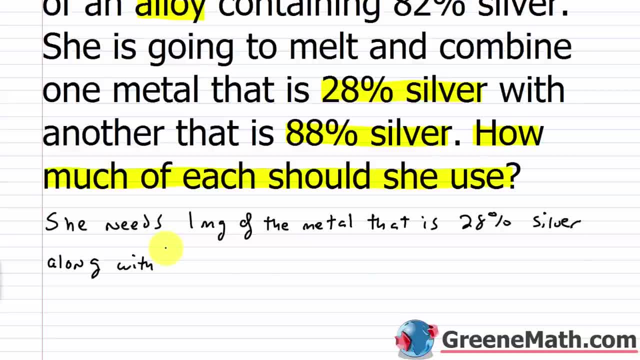 10, which is the total weight of this thing, minus 1, which is the weight of the metal that is 28% silver, so 9, so along with 9 milligrams, remember we set that up as 10 minus x. 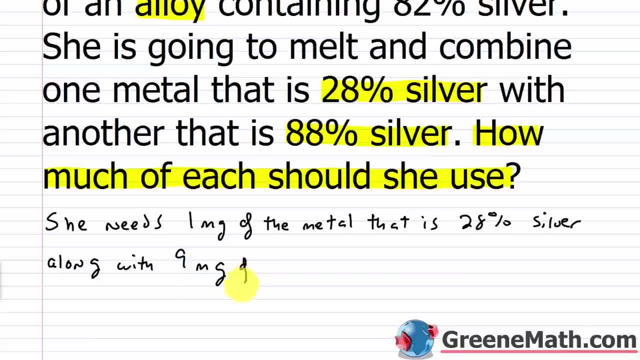 10 minus 1 would be 9. So along with 9 milligrams of the metal, 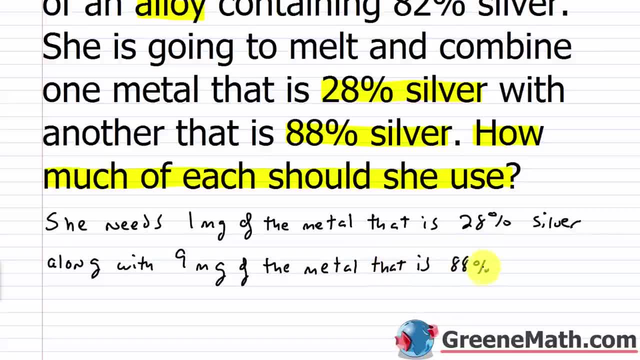 that is 88% silver. 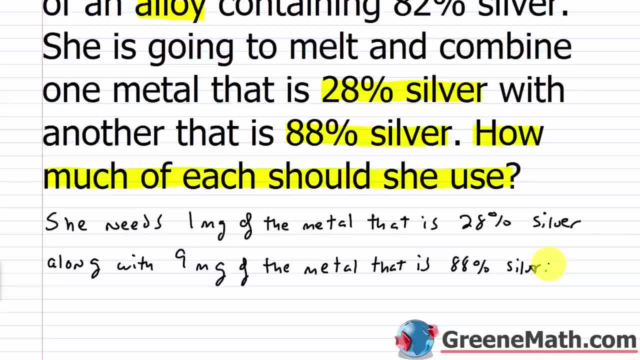 So that's what she's going to use to make this alloy that is 10 milligrams and 82% silver. So check 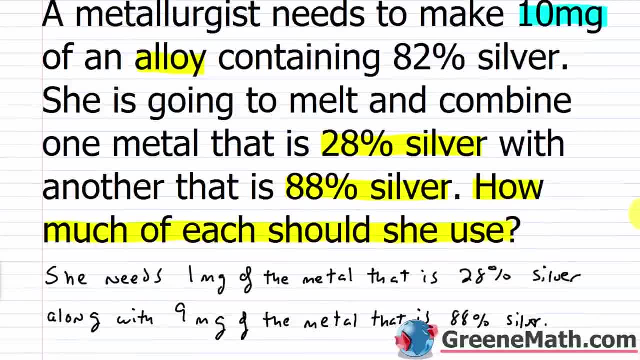 everything out. If you go back up, again, a metallurgist needs to make 10 milligrams of an alloy containing 82% silver. 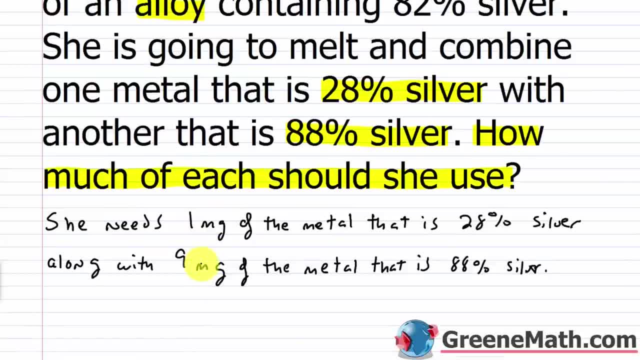 So, we know that 1 milligram plus 9 milligrams is 10 milligrams, so that part checks out. 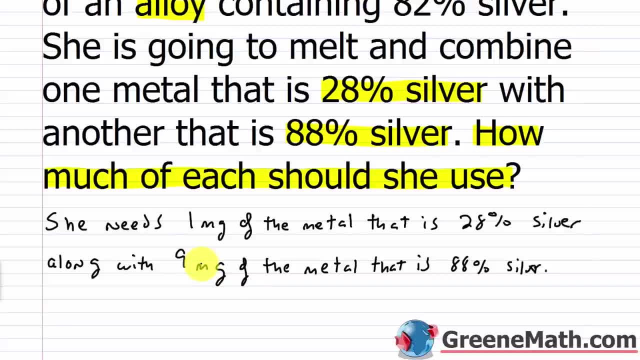 We just need to check the pure amount of silver in the substance. So our goal is to have 82%. It needs to be 82%. 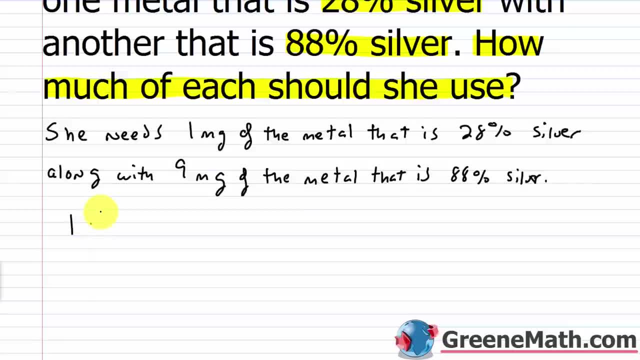 So if we have 1 milligram, that's 28% silver, times .28, and we add that to 9 milligrams, 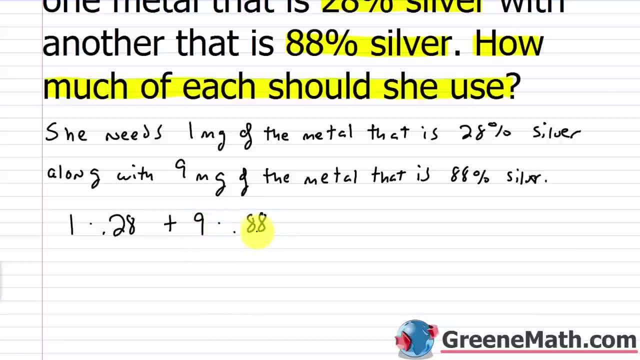 that's 88% silver, so times .88. 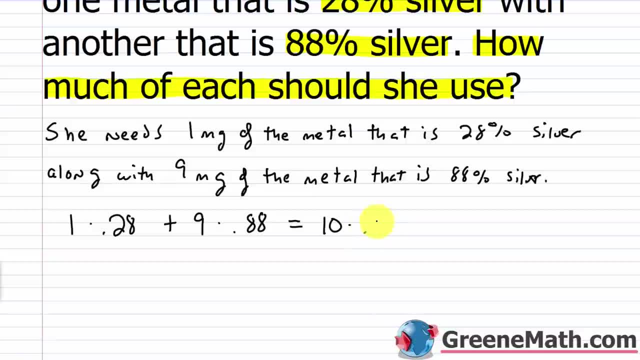 This should be equal to 10 milligrams times .82. And this is the exact equation that we set up. We just didn't know the values. So 1 times .28 is .28. And then plus, we have 9 times .88, that's 7.92. And again, 10 times .82 would be 8.2. So this is what I'm looking for. I'm looking for 8.2 milligrams of silver. In this 10 milligram 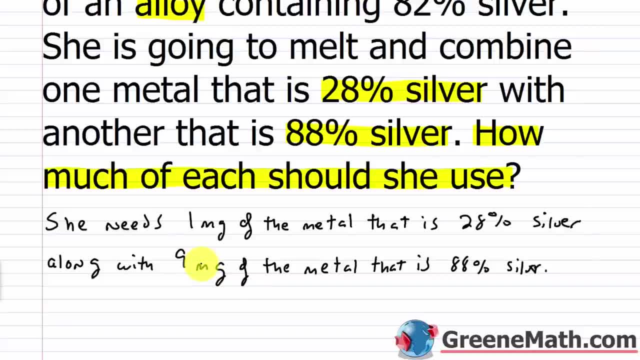 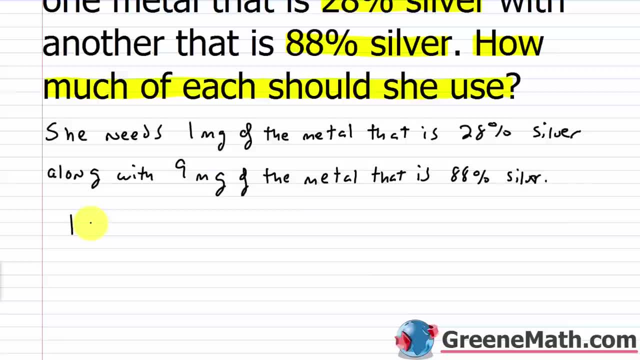 need to check the pure amount of silver in the substance. So our goal is to have 82%. It needs to be 82%. So if we have, We have 1 milligram, that's 28% silver times 0.28.. And we add that to 9 milligrams, that's 88% silver. so times 0.88.. This should be equal to 10 milligrams times 0.82.. 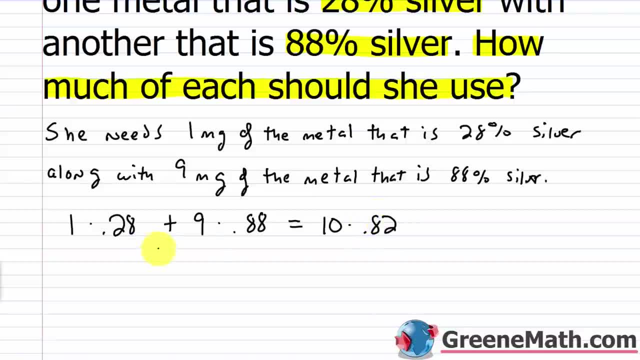 And this is the exact equation that we set up. We just didn't know the values. So 1 times 0.28 is 0.28.. And then, plus, we have 9 times 0.88,, that's 7.92.. 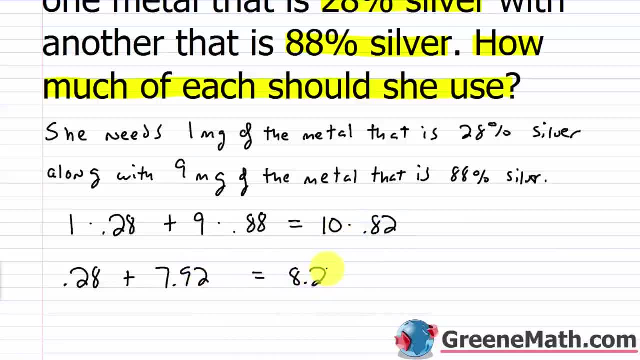 And again, 10 times 0.82 would be 8.2.. So this is what I'm looking for. I'm looking for 8.2 milligrams of silver in this 10 milligram alloy. So what is 0.28 plus 7.92?? Well, that is 8.2.. You get 8.2. 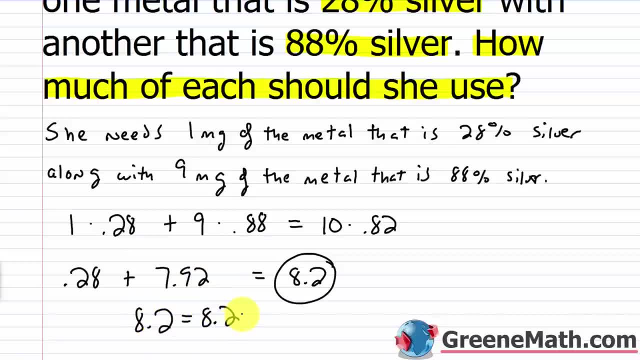 equals 8.2.. And so your answer here is correct. She needs to use 1 milligram of the metal. that is, 28% silver. She's going to have 0.28 milligrams of silver from that And then. 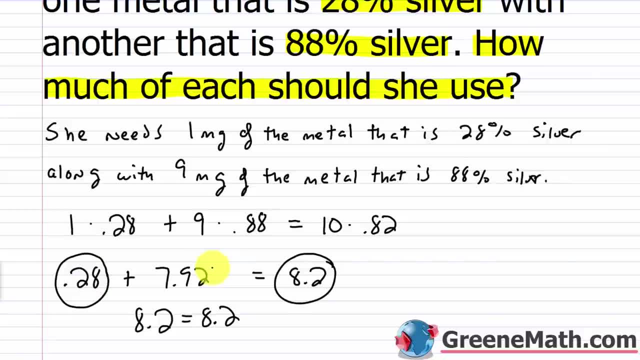 with 9 milligrams of the metal- that is 88% silver- She's going to get 7.92 milligrams of pure silver from that. She combines them together and she gets 8.2 milligrams of pure silver for her alloy. that is 82% silver. It's 8.2 milligrams out of a total of 10 milligrams. 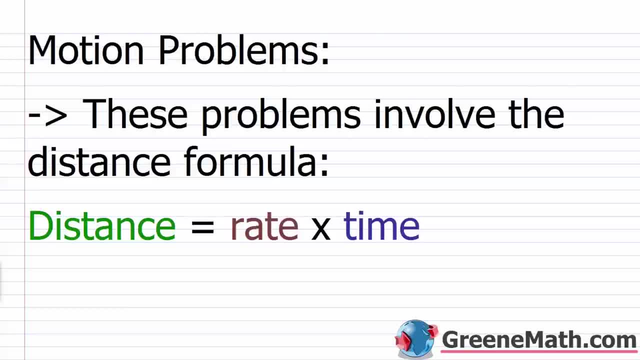 All right. So now we're going to talk a little bit about something known as motion problems. These problems involve the distance formula, And there's more than one distance formula. We're going to cover the other one in the last part of Algebra 1.. It relates to how 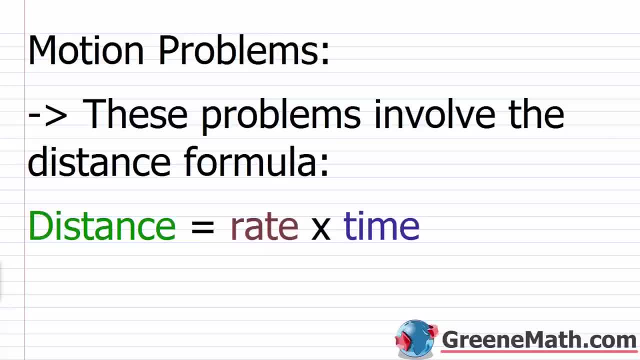 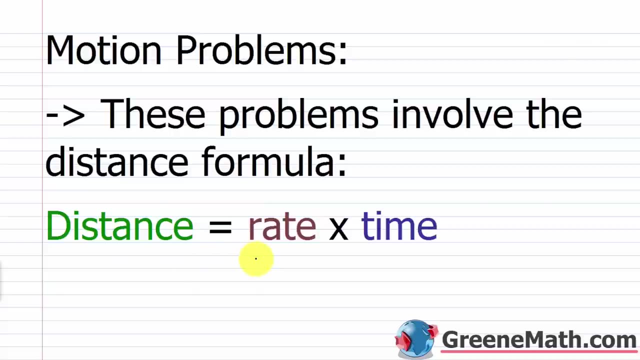 much distance is between two points on a graph. We're not talking about that one. We're talking about distance equals rate times time. so rate of speed times the amount of time traveled at that speed. And this formula is very, very intuitive. Pretty much everybody has taken. 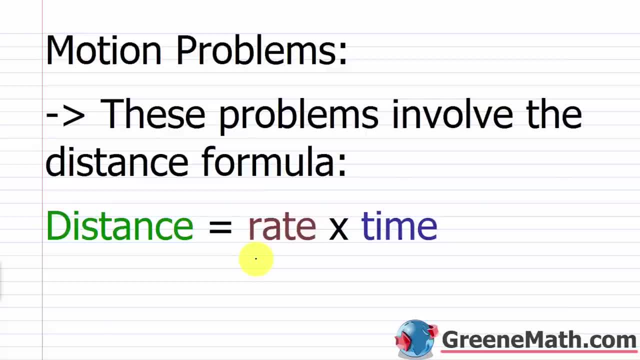 a road trip at some point and said: if we go 60 miles per hour for three hours, we're going to end up going 100 km, 180 miles. so in other words, if my rate of speed is 60 miles per hour, and this is in terms of hours, 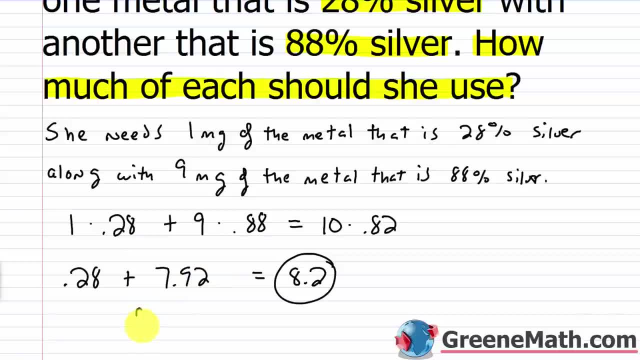 So what is .28 plus 7.92? Well, that is 8.2. You get 8.2 equals 8.2. And so your answer here is correct. 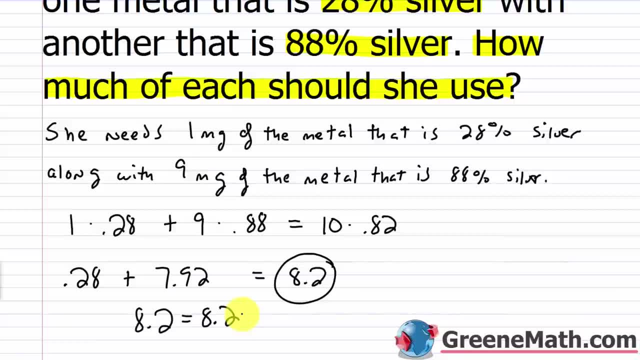 She needs to use 1 milligram of the metal that is 28% silver. She's going to have .28 milligrams of silver from 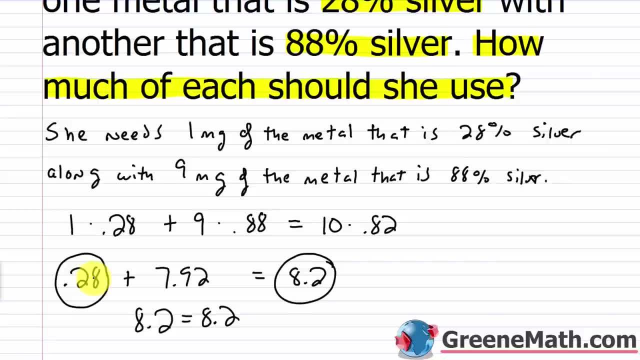 that. And then along with 9 milligrams of the metal that is 88% silver, she's going to get 7.92 milligrams of pure silver from that. 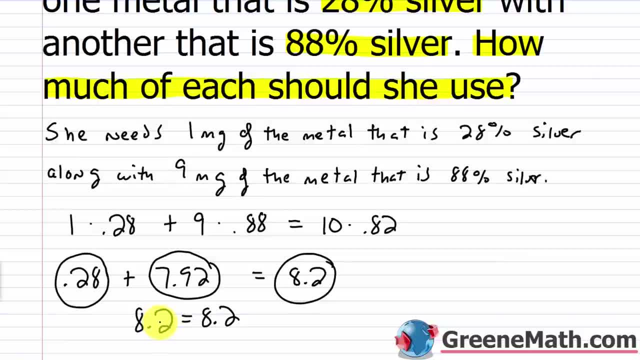 She combines them together and she gets 8.2 milligrams of pure silver for her alloy that is 82% silver. It's 8.2 milligrams out of a total of 10 milligrams. 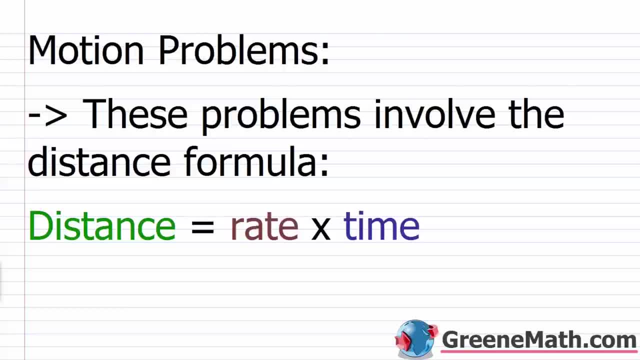 Alright, so now we're going to talk a little bit about something known as motion problems. These problems involve the distance formula. And there's more than one distance formula. We're going to cover the other one in the last part of Algebra 1. It relates to how much distance is between two points on a graph. We're not talking about 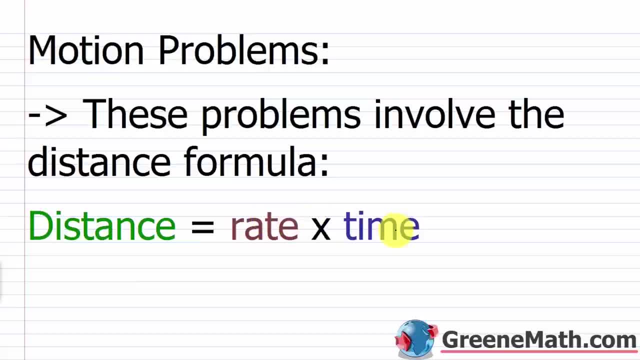 that one. We're talking about distance equals rate times time. 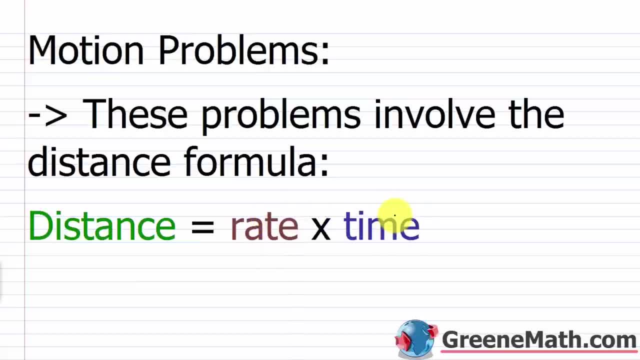 So, rate of speed times the amount of time traveled 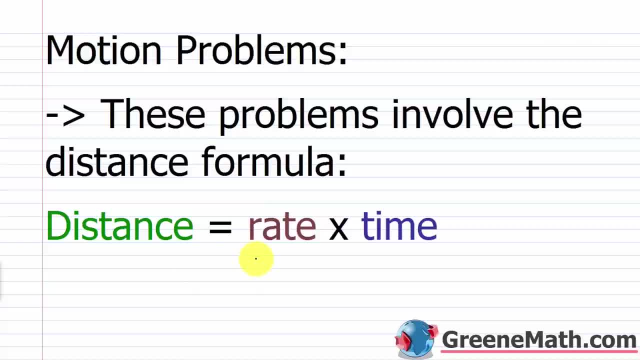 at that speed. And this formula is very, very intuitive. 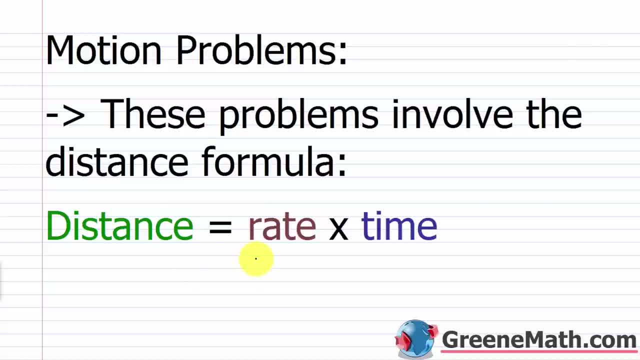 Pretty much everybody has taken a road trip at some point and said, if we go 60 miles per hour 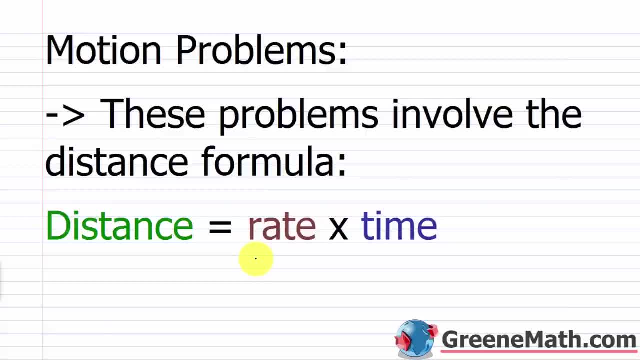 for three hours, we're going to end up going 180 miles. 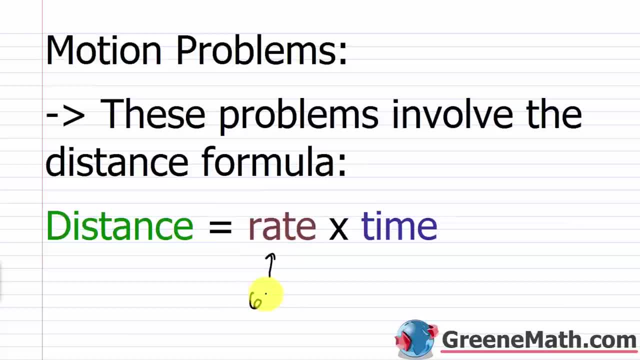 So, in other words, if my rate of speed is 60 miles per hour, and this is in terms of hours, so our time has to be given in terms of hours for this to make sense. So, 60 miles per hour times three hours, how far are we going to go? Well, forget about the units here. We're going 60 times three, that's 180. 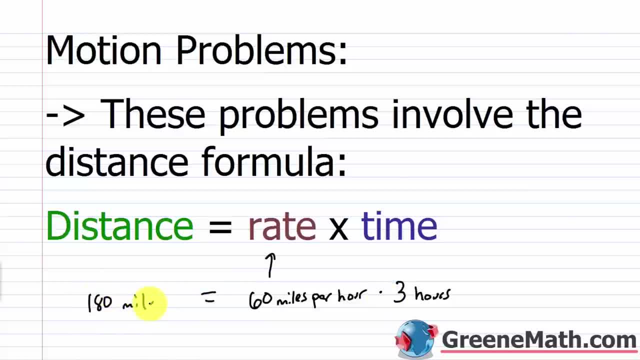 So, we're going to end up going 180 miles. 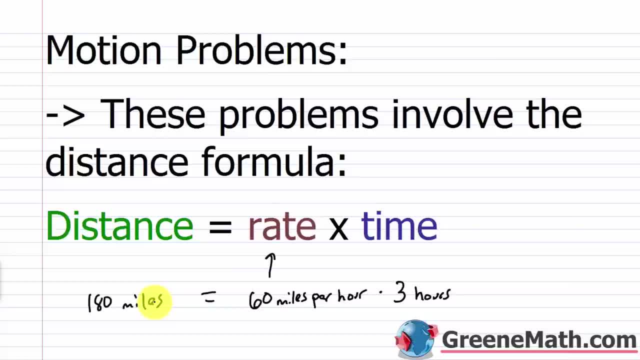 Right? If I go 60 miles per hour for three hours, we go 180 miles. We all know that. 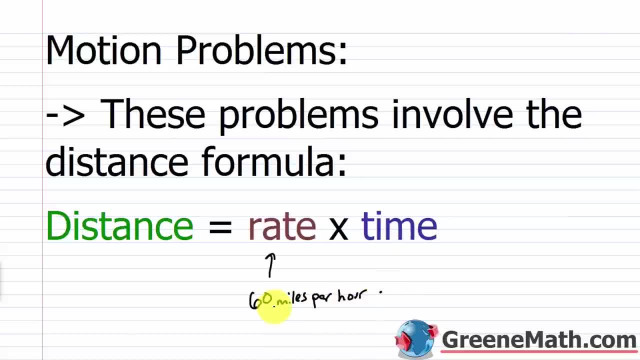 so our time has to be given in terms of hours for this to make sense. so 60 miles per hour times three hours, how far are we going to go? well, forget about the units here. we're going 60 times three, that's 180. so we're going to end up going 180 miles, right, if i go 60 miles per hour for three? 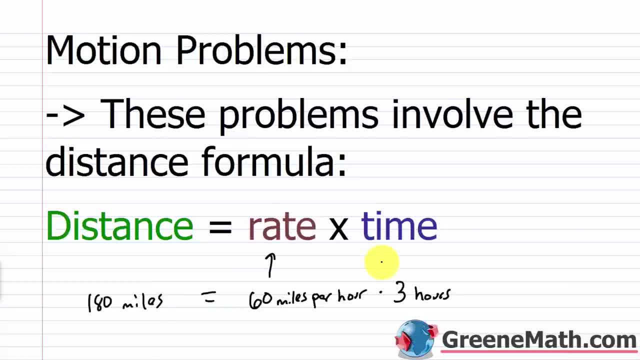 hours, we go 180 miles. we all know that. and that's what the distance formula does. it tells us that the amount of distance traveled is equal to the rate of speed times, the amount of time traveled. all right, so shannon left the science fair and traveled toward the recycling plant. 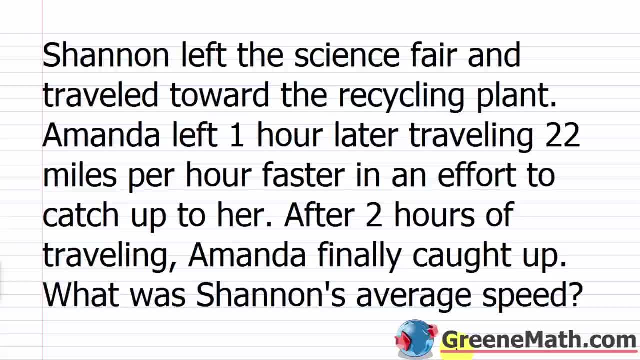 amanda left one hour later, traveling 22 miles per hour faster, in an effort to catch up to her. after two hours of traveling, amanda finally caught up. what was shannon's average speed? here's the key question here: what was shannon's average speed? i can tell you, this is: 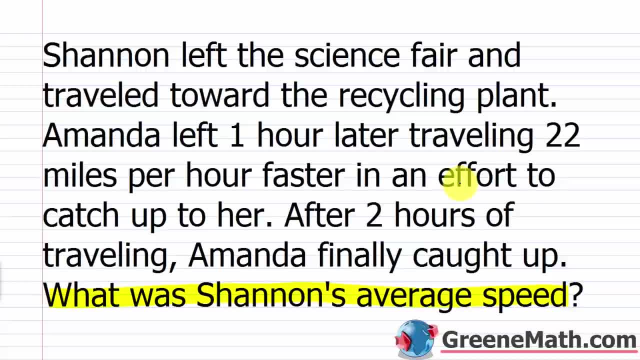 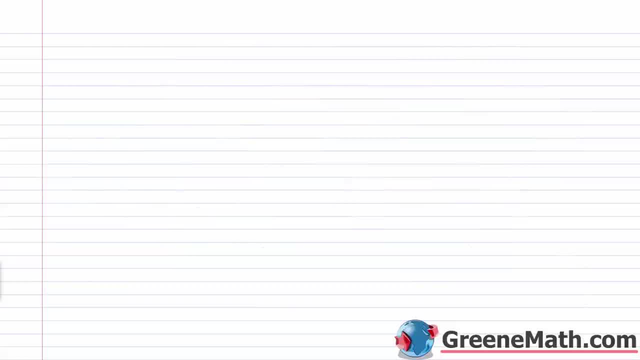 kind of a difficult problem to solve. if you've never done a motion ward problem right, you really have a lot of things that you have to consider here. so the first thing is, let's revisit our distance formula. so distance is, is is the rate of speed times the time traveled. 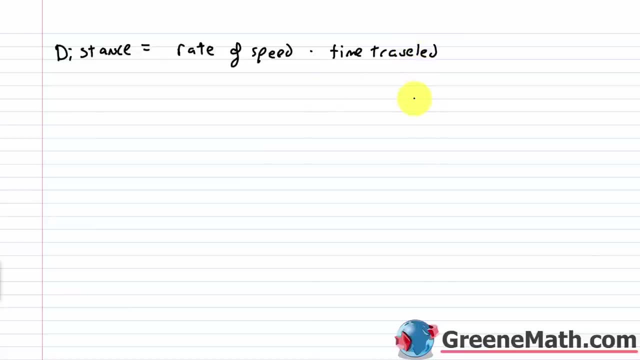 and again. if you ever forget that, just think about: okay, i'm taking a road trip and i'm going for two hours. that's my time times. 50 miles per hour, that's my rate of speed. that gives me a distance. so in that case 100 is equal to rate of speed of 50 times time traveled. 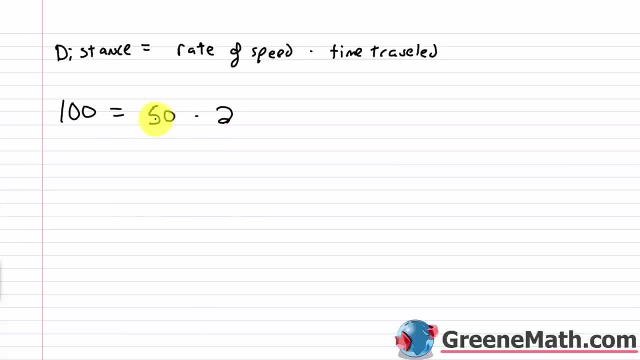 two, and i like to call this the rate of speed of 50 times the time traveled. two, and i like to call this the rate of speed of 50 times the time traveled. two the units out just for simplicity. but this is 50 miles per hour, this is two hours, this is 100. 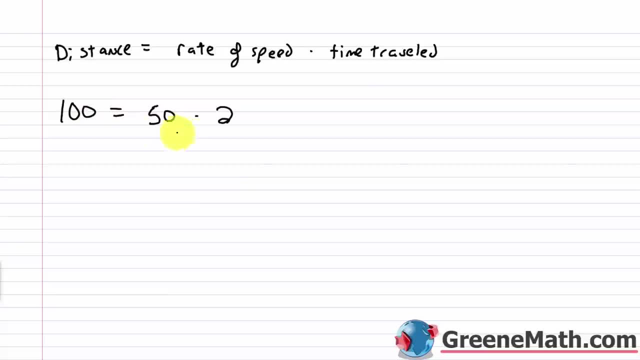 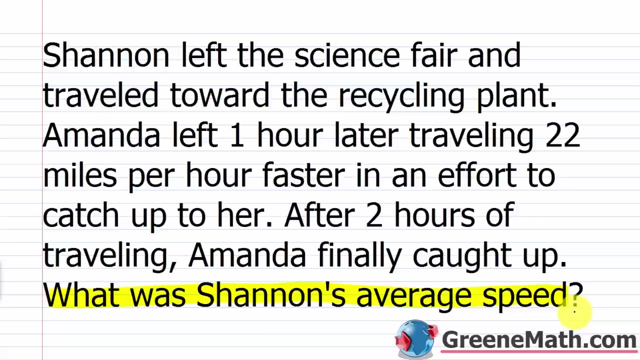 miles. now you see that one side equals the other. so if i have a rate of speed and a time traveled, i have a distance and i can calculate that. now, knowing this information here, if we go back up to the problem, kind of the first thing we're given is that shanna left the science fair and traveled. 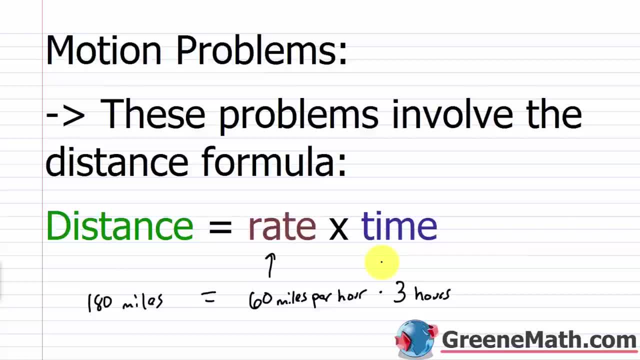 And that's what the distance formula does. It tells us that the amount of distance traveled is equal to the rate of speed times the amount of time traveled. 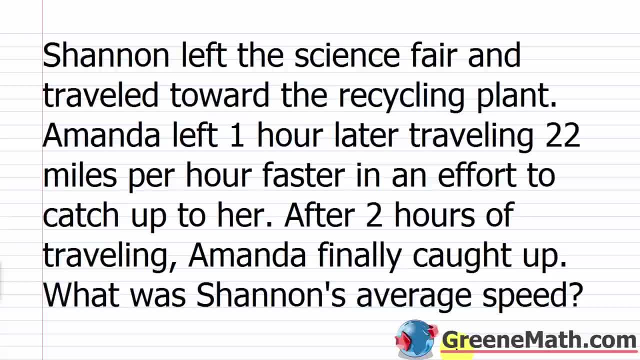 Alright, so Shannon left the science fair and traveled toward the recycling plant. Amanda left one hour later, traveling 22 miles per hour faster in an effort to catch up to her. After two hours of traveling, Amanda finally caught up. 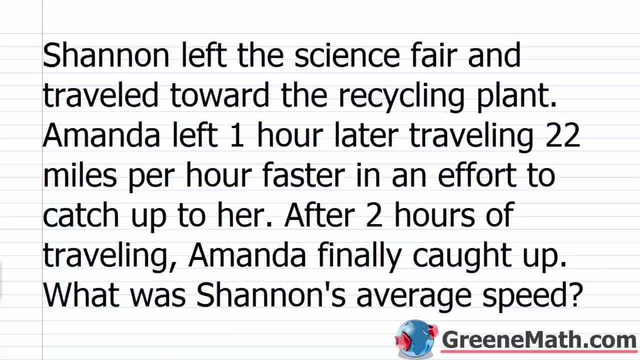 What was Shannon's average speed? Here's the key question here. 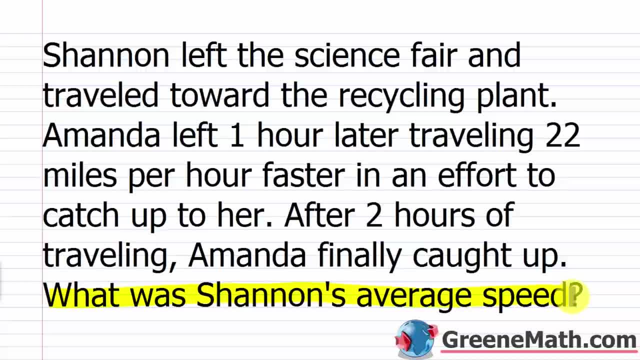 What was Shannon's average speed? Now, I can tell you this is kind of a difficult problem to solve if you've never done a motion ward problem, right? You really have a lot of things that you have to consider here. So, the first thing is, let's 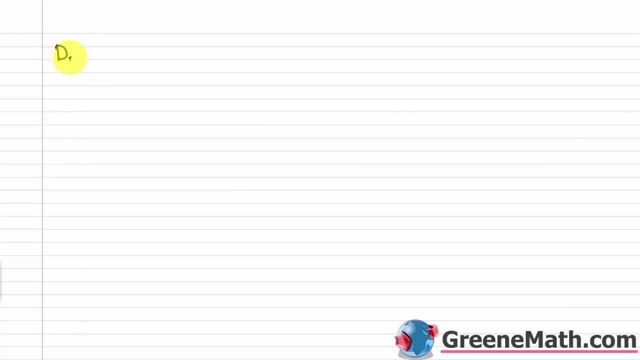 revisit our distance formula. So, distance 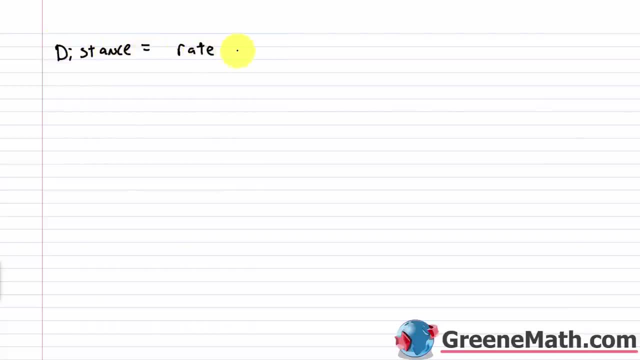 is equal to the rate of speed times the time traveled. 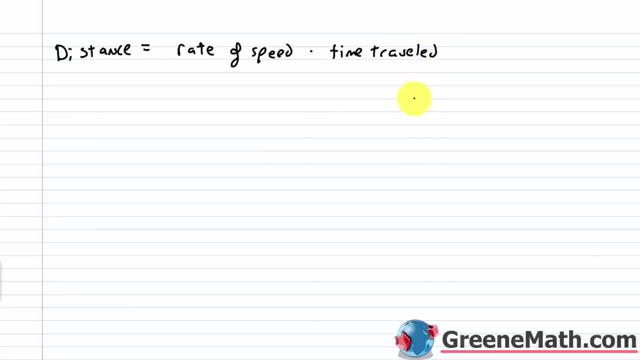 And again, if you ever forget that, just think about okay, I'm taking a road trip and I'm going for two hours, that's my time, times 50 miles per hour, that's my rate of speed, that gives me a distance. So, in that case, 100 is equal to rate of speed of 50 times time traveled, 2. 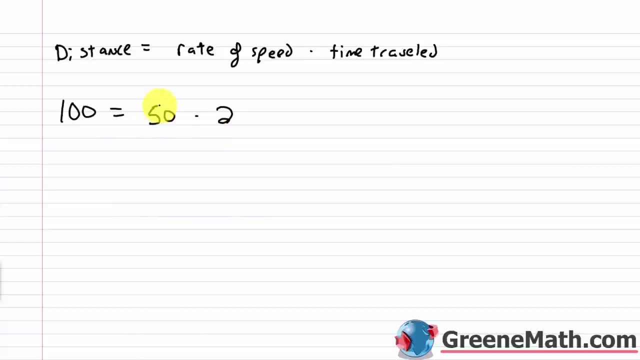 And I left the units out just for simplicity, but this is 50 miles per hour, this is 2 hours, this is 100 miles. 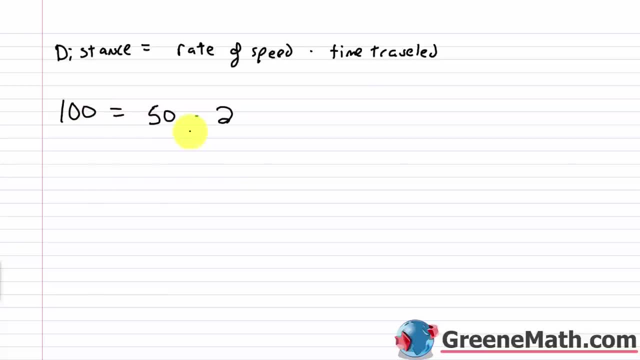 Now, you see that one side equals the other. 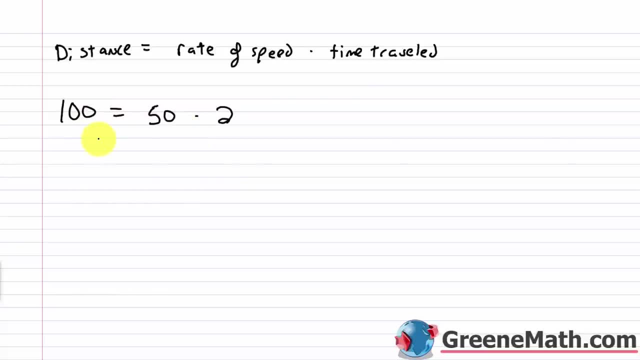 So, if I have a rate of speed and a time traveled, I have a distance. And I can calculate that. 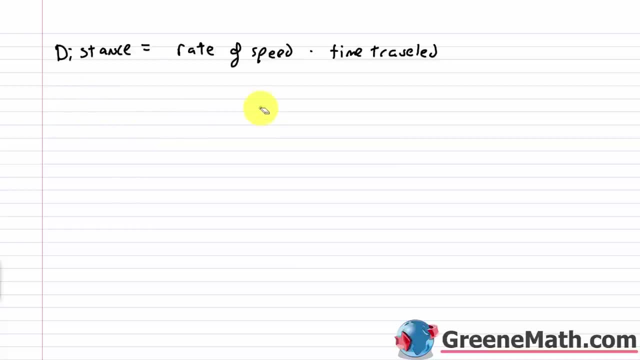 Now, knowing this information here, if we go back up to the problem, 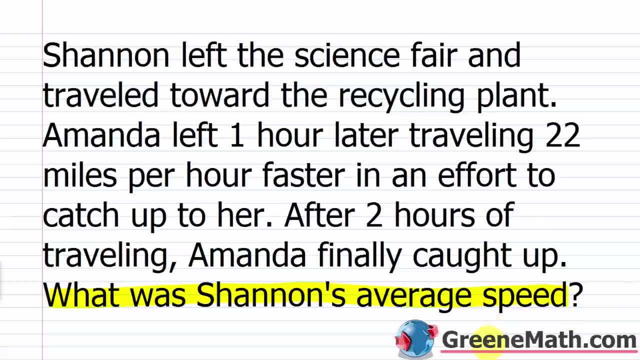 kind of the first thing we're given is that Shanna left the science fair and traveled towards the recycling plant. It doesn't give us a distance. 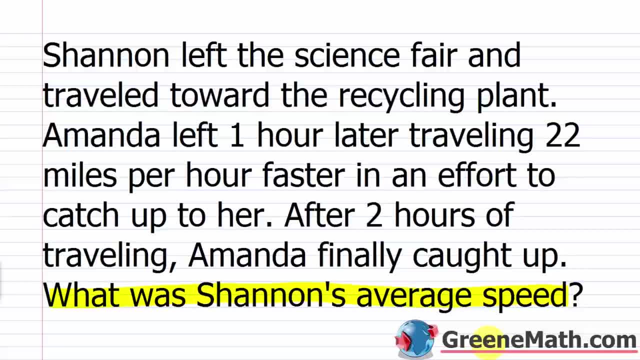 Amanda left one hour later, traveling 22 miles per hour faster in an effort to catch up to her. After 2 hours, so this is key, after 2 hours of traveling, Amanda finally caught up. 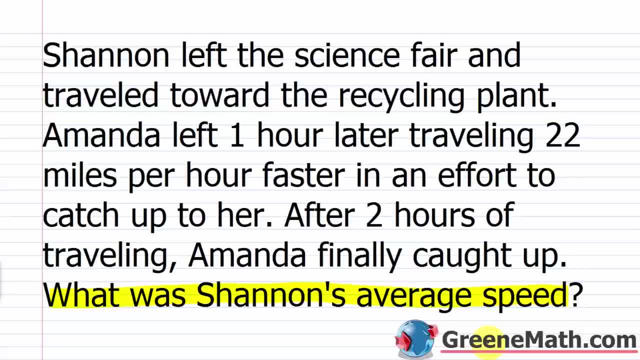 towards the recycling plant. it doesn't give us a distance. the science fair and traveled towards the recycling plant. it doesn't give us a distance. amanda left one hour later, traveling 22 miles per hour faster in an effort to catch up to her after two hours. so this is key: after two hours of traveling, amanda finally caught up. 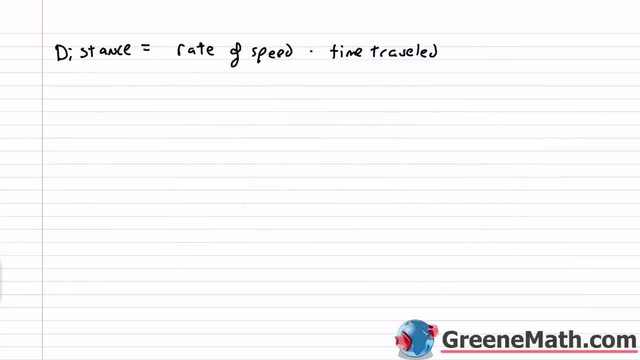 so one thing we know about the distance: in this particular case, amanda and shannon travel the same amount or travel the same distance, so their distances in the end will be equal. now, later on, in algebra we use some different types of notation which won't come up for a while, but i'm going to write d, a capital d, with a small a. 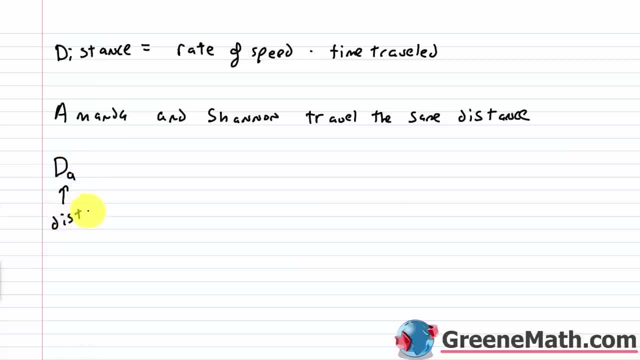 to relate the amount of distance. this is the distance for amanda and this is equal to- i'm going to put a big d with a little s- and this is the distance for shannon. and this is just here to show you that these two distances are equal. they both leave from. 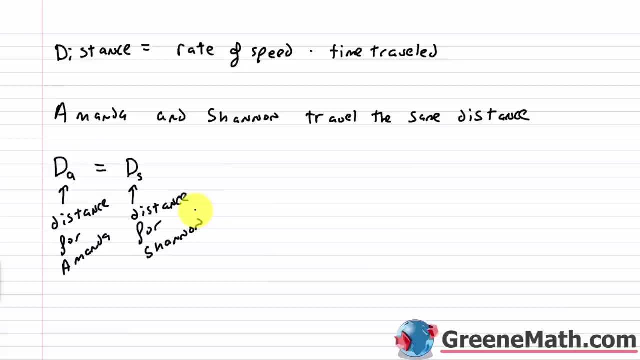 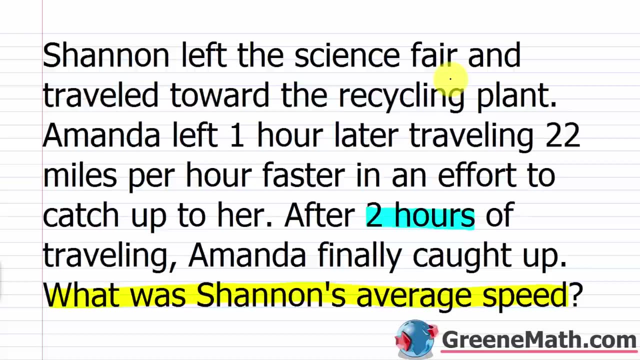 the same place and they both go to the same place. now they doiek to say that my distance between them do it in a different amount of time and so they do it at different rates as well. so the time is different and the rate of speed is different, but the distances are the same. so that's the first. 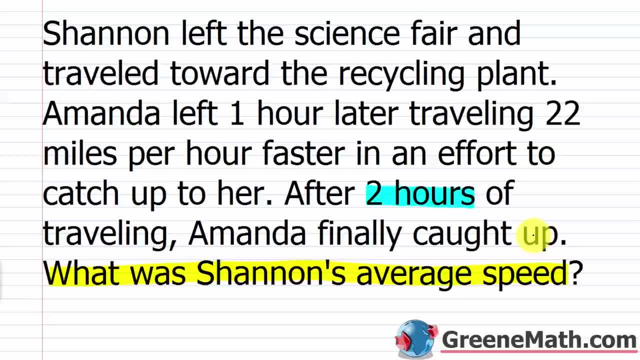 thing. so let's talk a little bit about time now. so shannon left the science fair and traveled toward the recycling plant. amanda left one hour later, so whatever amount of time that shannon drives, for, it's an hour more than amanda, because amanda delayed her trip by an hour. 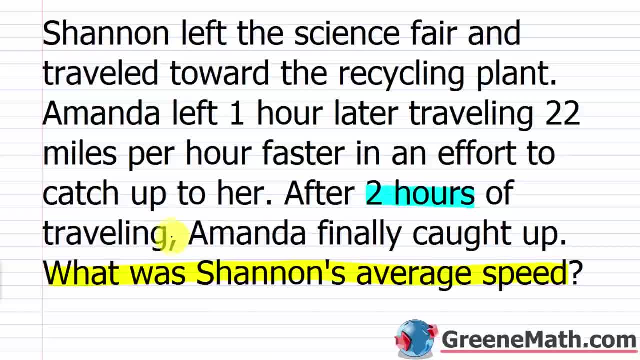 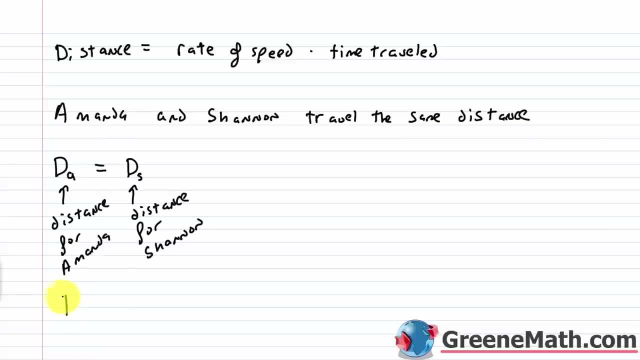 so it says here: after two hours of traveling, amanda finally caught up. if amanda drives for two hours and she drove for an hour less than shannon, then shannon drove for three hours. so when we talk about time, let's put a big t and a little a, and this is the time for amanda. 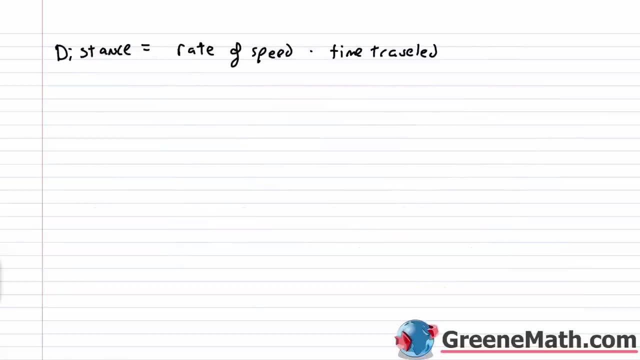 So, one thing we know about the distance, in this particular case, Amanda and Shannon travel the same amount. Or travel the same distance. 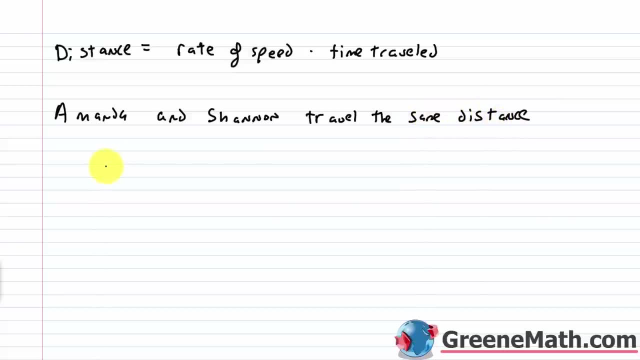 So, their distances in the end will be equal. Now, later on in algebra, we use some different types of notation, which won't come up for a while, but I'm going to write D, a capital D, with a small a to relate the amount of distance, this is the distance for Amanda. 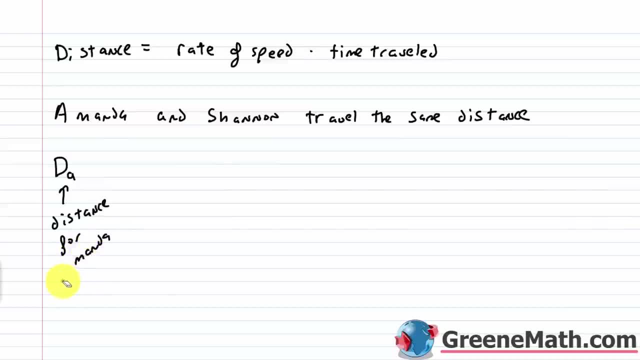 And this is equal to, I'm going to put a big D with a little s, and this is the distance for Shannon. 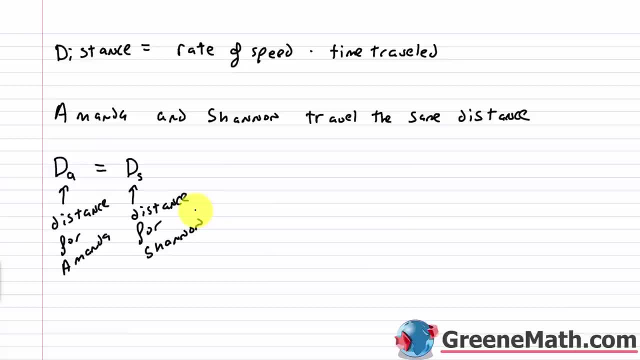 And this is just here to show you that these two distances are equal. They both leave from the same place, and they both go to the same place. 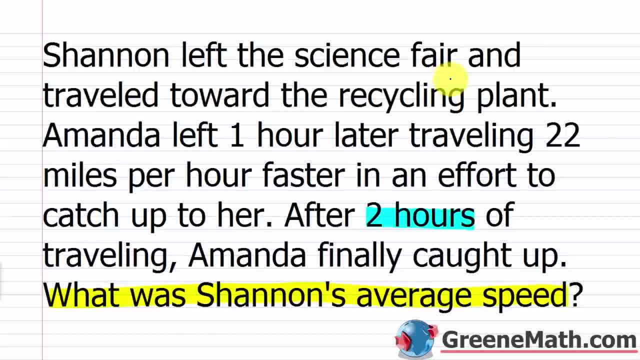 Now, they do it in a different amount of time, and so they do it at different rates as well. 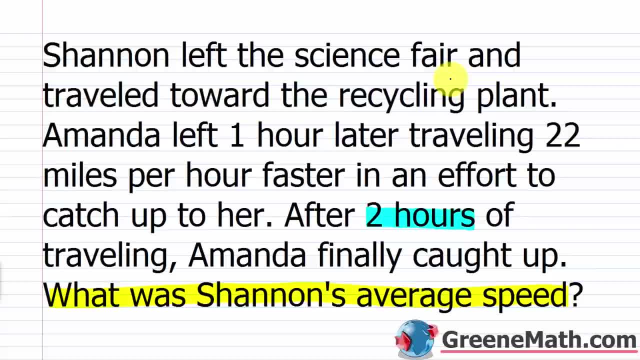 So, the time is different, and the rate of speed is different, but the distances are the same. So, that's the first thing. So, let's talk a little bit about time now. 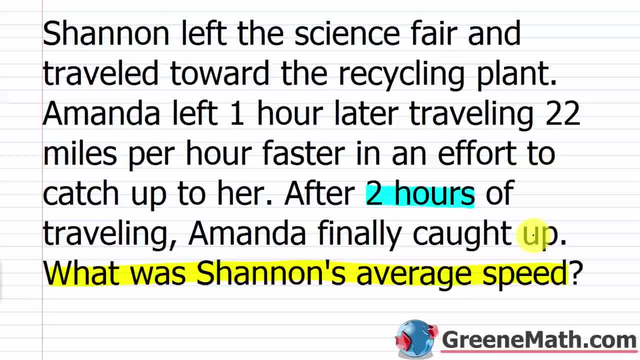 So, Shannon left the science fair and traveled toward the recycling plant. Amanda left one hour later. So, whatever amount of time that Shannon drives for, it's an hour more than Amanda, because Amanda delayed her trip by an hour. 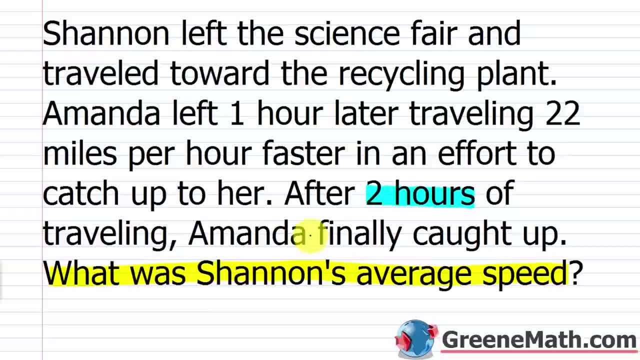 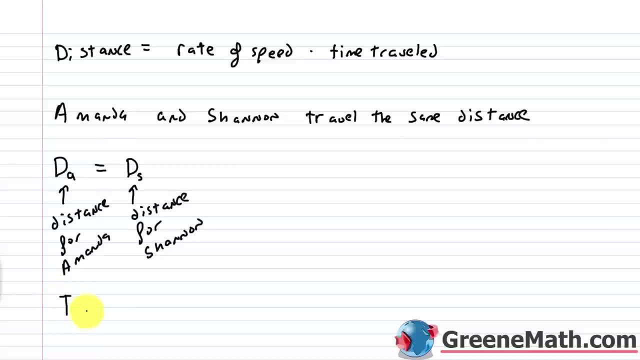 So, it says here after two hours of traveling, Amanda finally caught up. If Amanda drives for two hours, and she drove for an hour less than Shannon, then Shannon drove for three hours. So, when we talk about time, let's put a big T and a little a, and this is the time for Amanda. Time for Amanda. 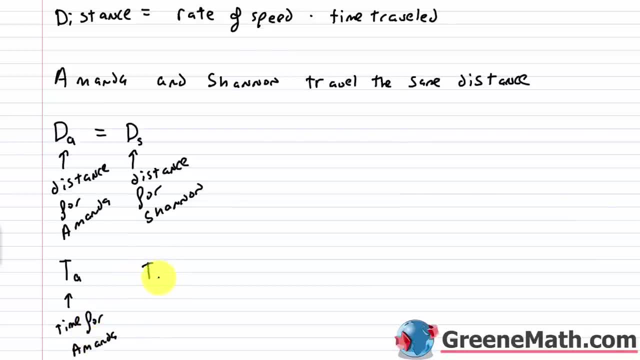 Let's put a big T and a little s, and this is the time for Shannon. 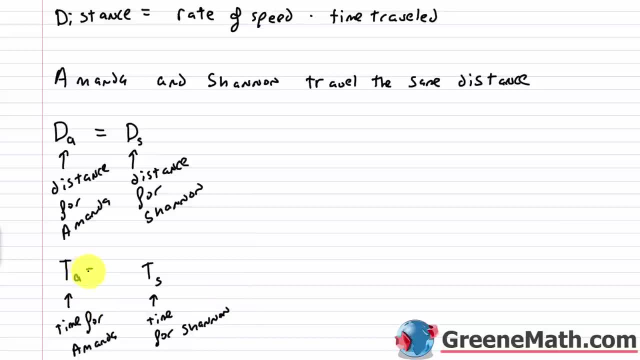 And we know the time for Amanda is two hours. 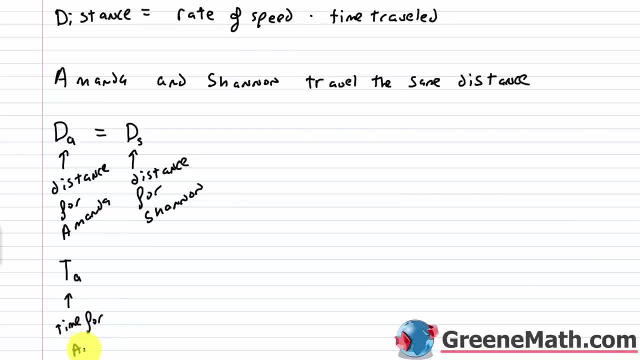 time. let's put a big t and a little s and this is the time for shannon, and we know the time for amanda is two hours. we know the time for shannon is one more hour than that, so three hours. i just put two and then three. just need to get some information. 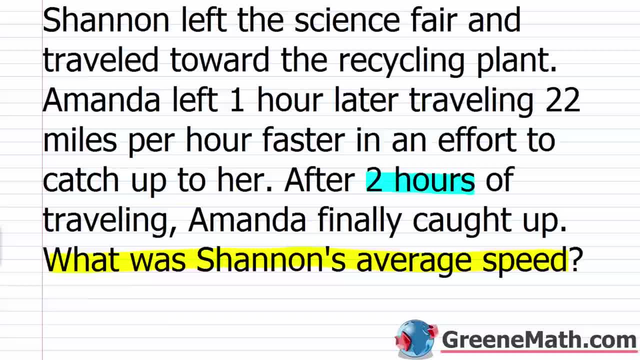 about the rate of speed. so shannon left the science fair and traveled toward the recycling plant. amanda left one hour later, traveling 22 miles per hour faster, in an effort to catch up to her. now, what i can do here, since amanda is going 22 miles per hour faster, i don't. 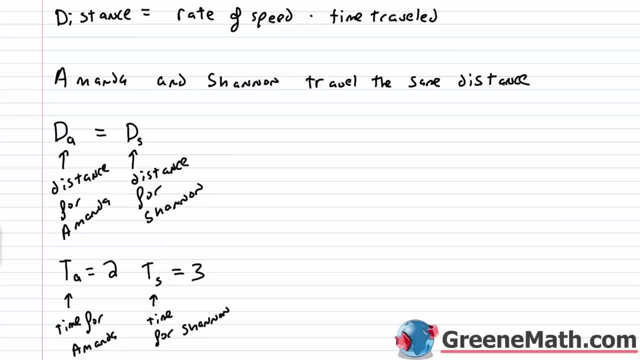 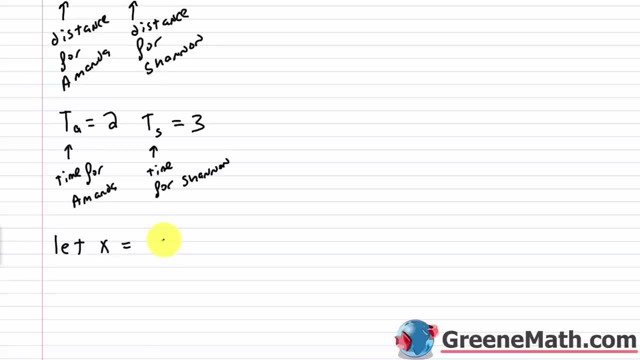 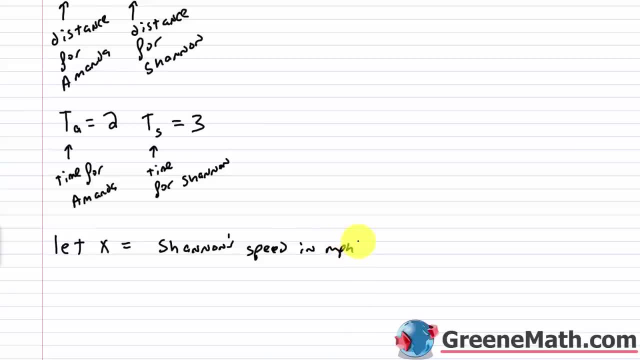 so let's let x equal shannon's speed in miles per hour. so then x plus 22, as it tells us in the problem she she's going 22 miles per hour faster amanda is is going to equal amanda speed. again, this is in miles per hour. so we have a little bit more information. let me scroll down. 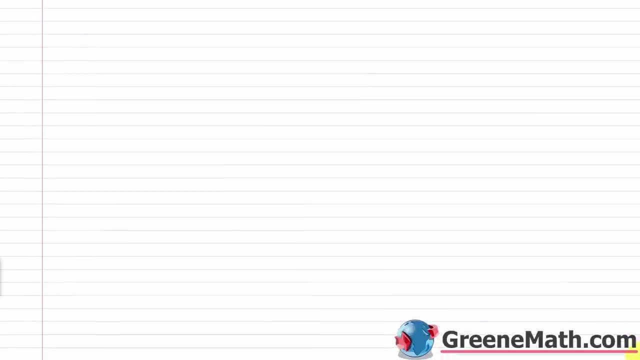 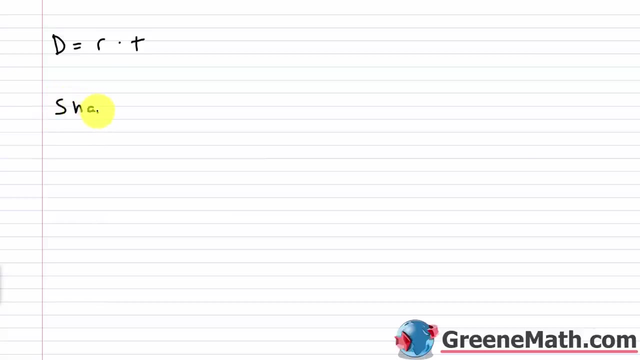 and get a little room. we know from the distance formula, again, distance is equal to rate of speed, times, time traveled. so for shannon, what information? do we have her distance, we have her rate of speed, which i assigned the variable x to, and we have her time as three for three hours. so distance for her equals 3x. now for amanda. 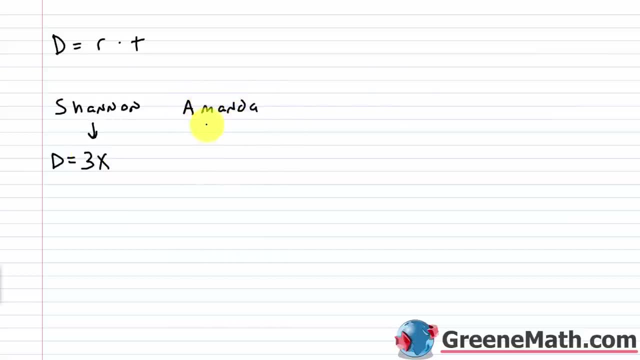 her distance looks like this: she has a time traveled of two hours and her rate of speed is x plus 22. remember: x plus 22 is the rate of speed, so the whole thing has to be multiplied by two. if you don't use parentheses, this just looks like 2x plus 22. that's wrong. the two has to be. 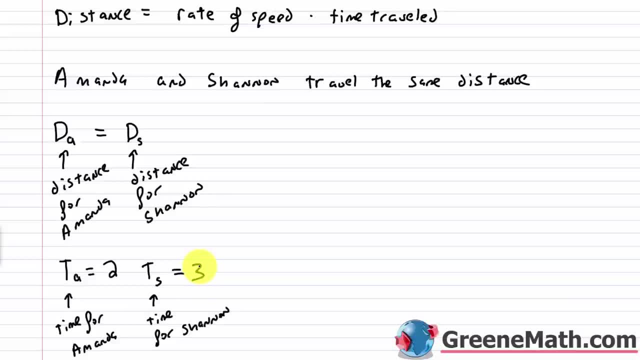 We know the time for Shannon is one more hour than that, so three hours. We just need to get some information about the rate of speed. 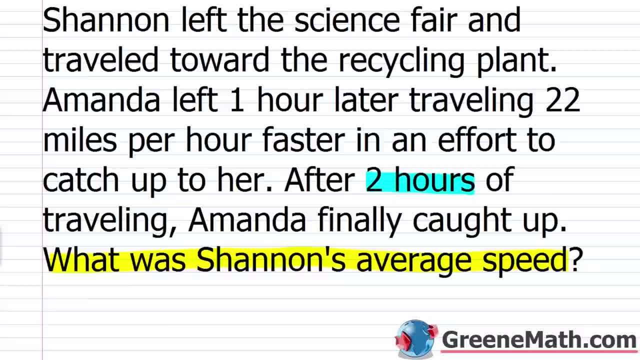 So, Shannon left the science fair and traveled toward the recycling plant. Amanda left one hour later, traveling 22 miles per hour faster in an effort to catch up to her. 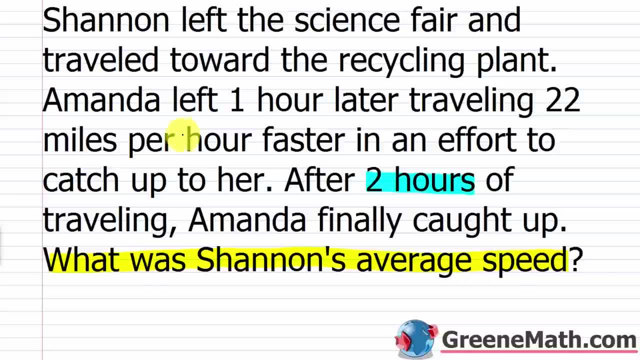 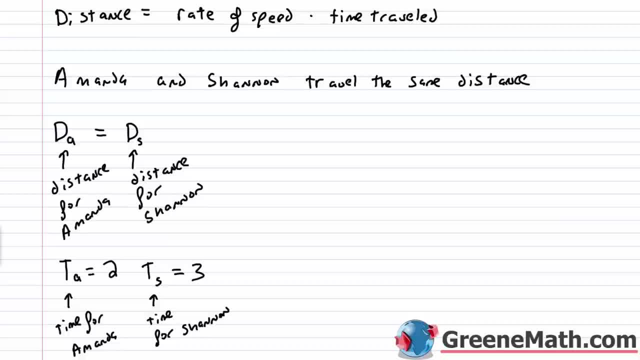 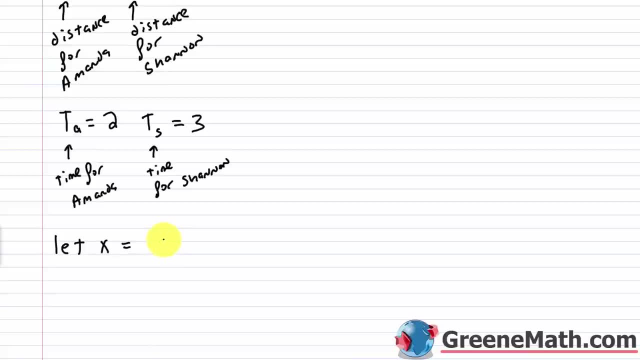 Now, what I can do here, since Amanda is going 22 miles per hour faster, I don't know how fast Shannon's going. So, I can use a variable to represent that. So, let's let x let's let x equal Shannon's speed in miles per hour. 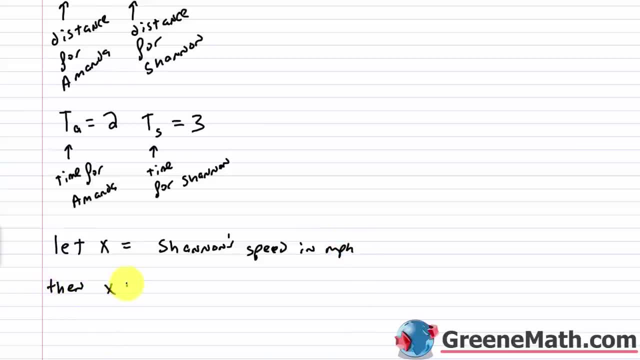 So, then x plus 22 as it tells us in the problem, she's going 22 miles per hour faster. Amanda is going to equal Amanda's speed. 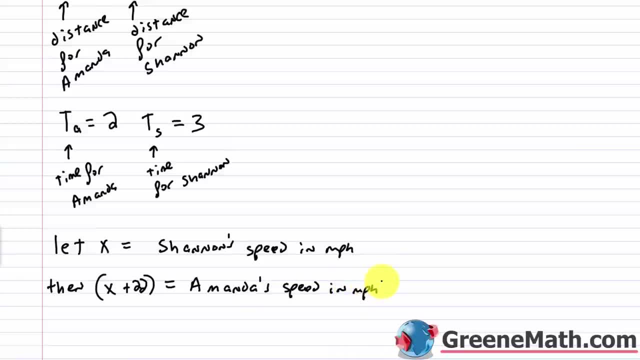 Again, this is in miles per hour. So, we have a little bit more information. 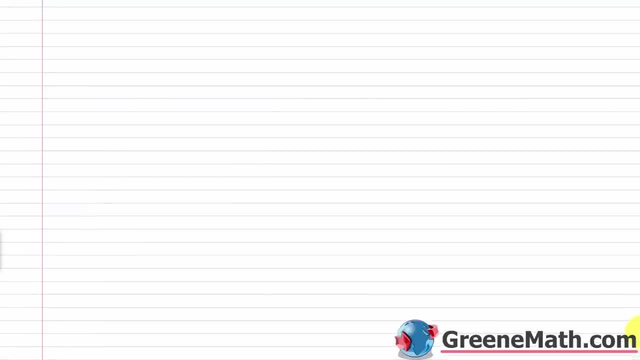 Let me scroll down and get a little room. We know from the distance formula, again, 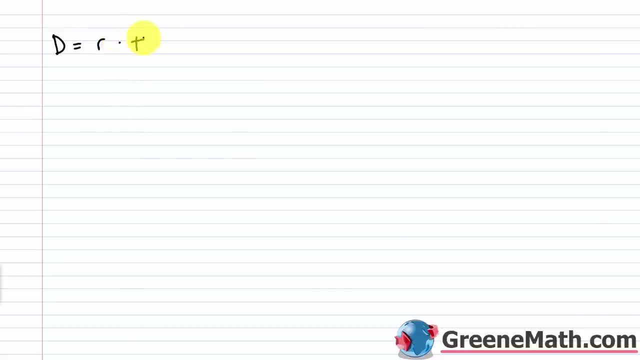 distance is equal to rate of speed times time traveled. 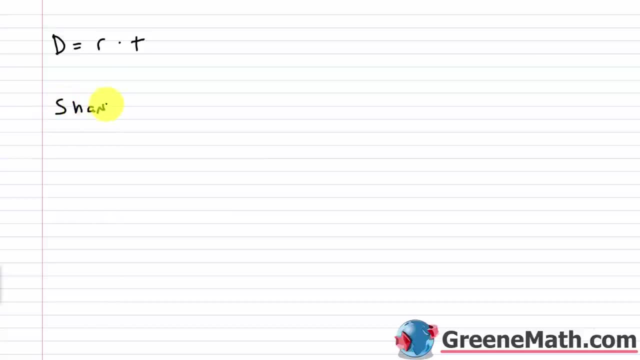 So, for Shannon, Shannon 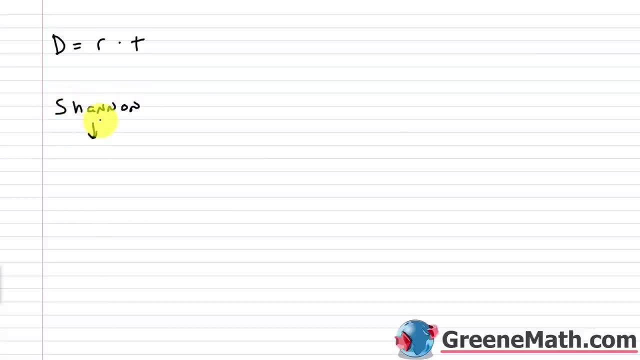 what information do we have? 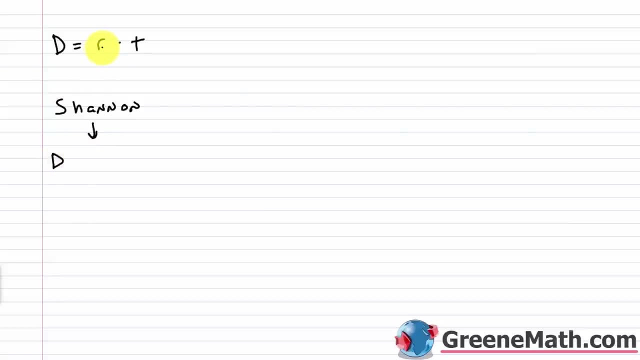 Her distance, we have her rate of speed, which I assigned the variable x to, and we have her time as 3 for 3 hours. 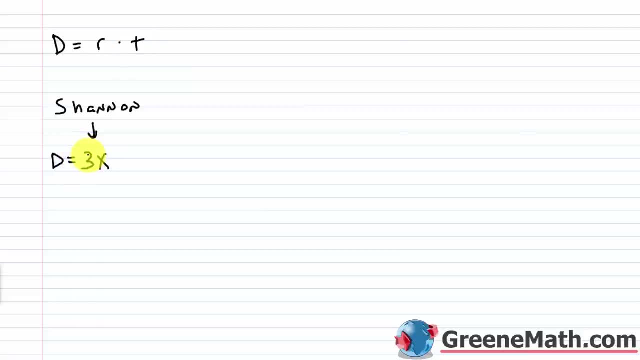 So, distance for her equals 3x. Now, for Amanda, 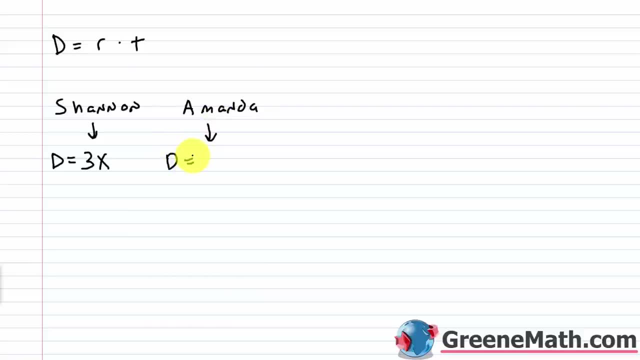 her distance looks like this. She has a time traveled of 2 hours, and her rate of speed is x plus 22. Remember, x plus 22 is the rate of speed, so the whole thing has to be multiplied by 2. 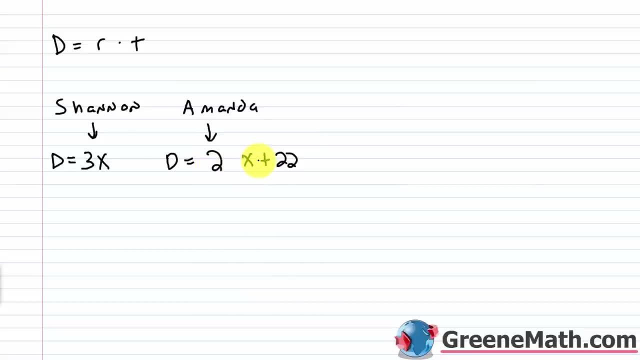 If you don't use parentheses, this just looks like 2x plus 22. 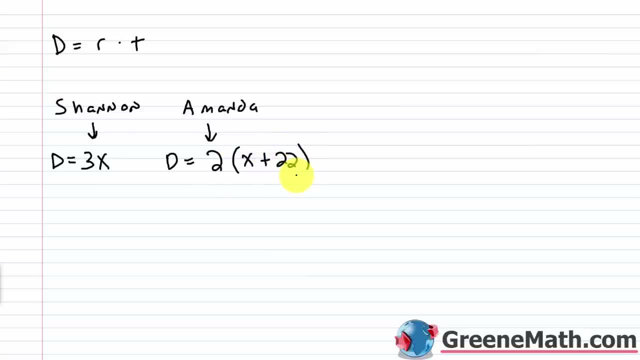 That's wrong. The 2 has to be multiplied by the entire thing, each term. 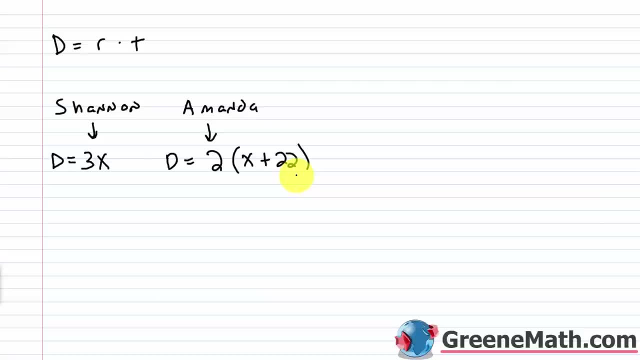 So, we have a distance for each person 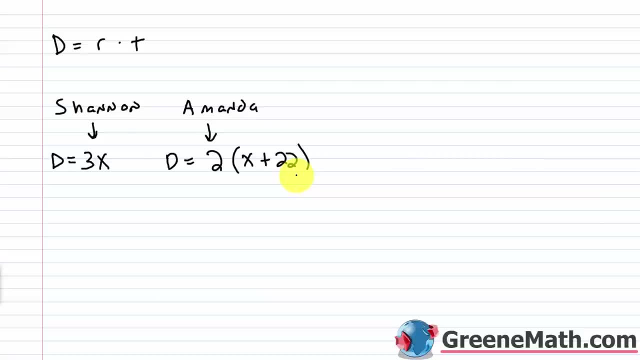 individually, and remember the two distances are the same. 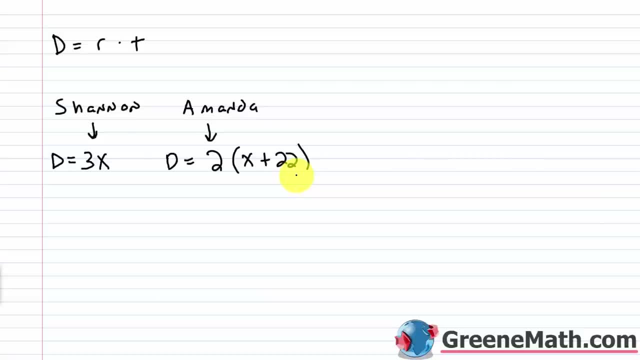 So, this is how we get our equation in this type of problem. 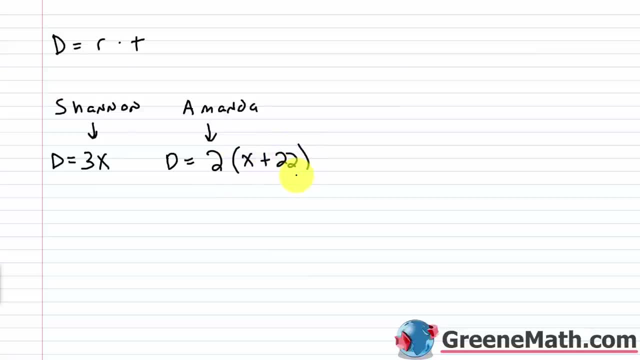 multiplied by the entire thing each term. so we have we have a distance for each person individually, and remember the two distances are the same. so this is how we get our equation in this type of problem. we know that Shannon's distance. okay, remember, I put d with a little. 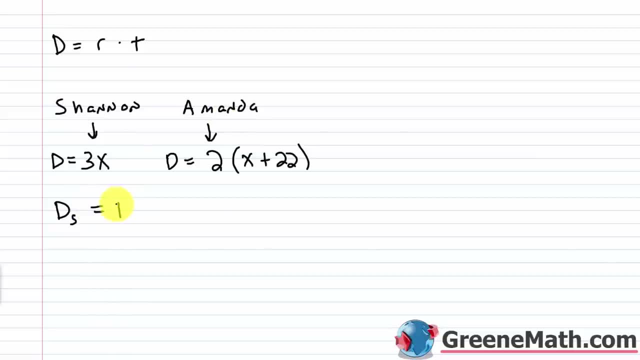 s for Shannon's distance is equal to Amanda's distance d with a little a, so I can take 3x, which relates to to Shannon's distance 3x, and I can set that equal to 2 times the quantity x plus 22.. Remember. 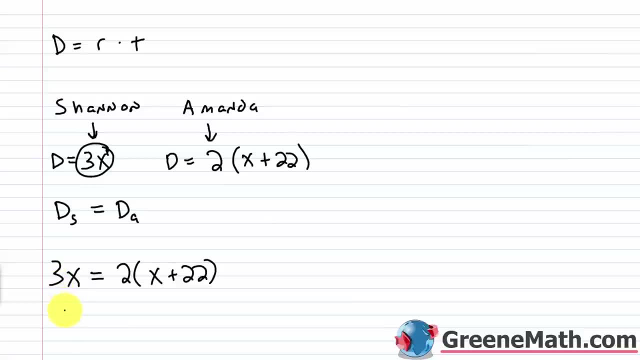 if you give me a rate times a time, I have a distance, So I have a rate times a time here. that's a distance, and it's equal to or the same as a rate times a time here, which is another distance. right, These two distances are the same. They look different because the time and the rates. 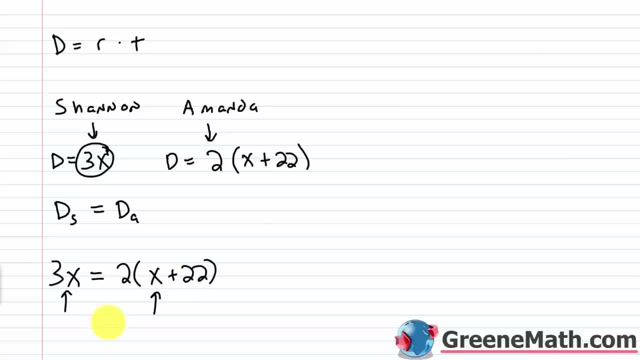 are different, but in the end they're the same. So what I can do now is just solve this equation and find out rates of speed. So over here I'm going to simplify: 2 times: x is 2x plus 2 times. 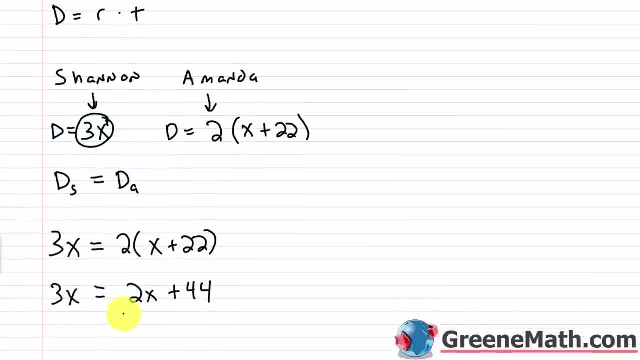 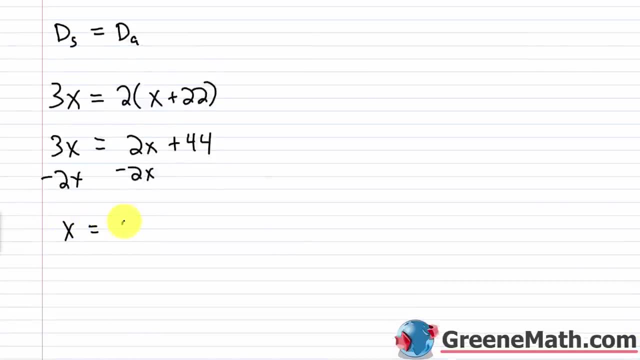 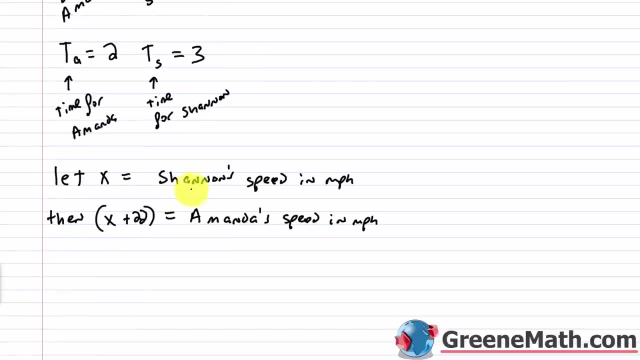 22,, that's 44. Over here I have 3x Subtract, 2x away from each side. Very, very simple equation We end up with: x is equal to 44. Remember 44 was the rate of speed for Shannon. Let x equal. 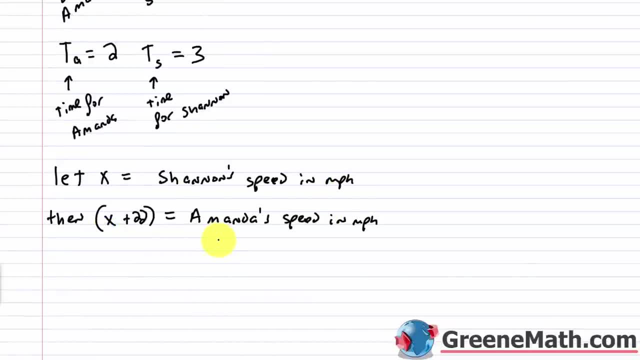 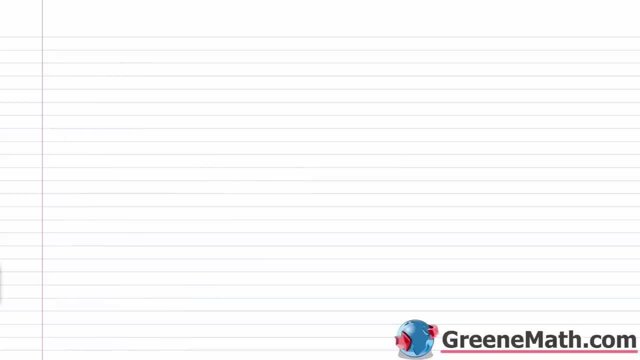 Shannon's speed in miles per hour. Then x plus 22, or 44 plus 22, or 66, is Amanda's speed in miles per hour. So let's go ahead and write our answer. So what was Shannon's average speed? is our official question. So Shannon's average speed. 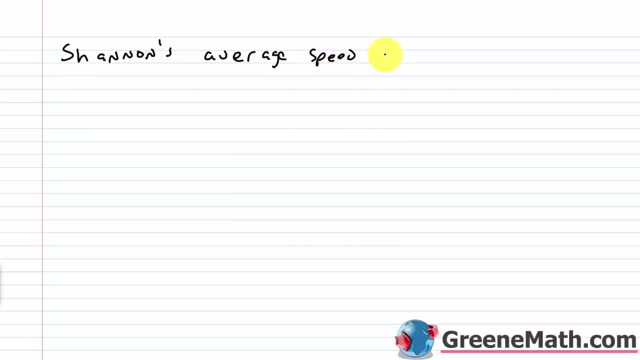 was 44 miles per hour, And we can check this to make sure that it's true. So we know that Shannon traveled for three hours. So three hours, think about your road trip. Three hours times 44 miles per hour, How far am I going to go? I'm going to go 132 miles. 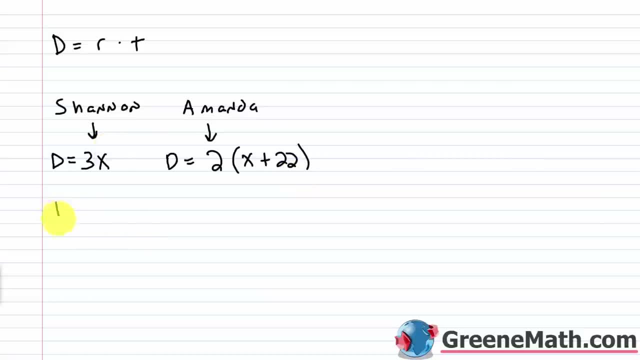 We know that Shannon's distance, remember I put d with a little s for Shannon's distance, is equal to Amanda's distance, d with a little a. So, I can take 3x, which relates to Shannon's distance, 3x, and I can set that equal to 2 times the quantity x plus 22. 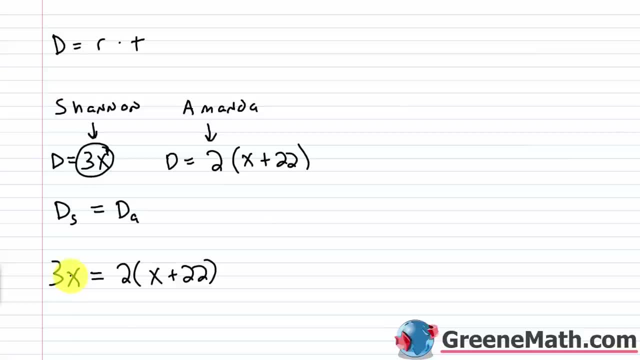 Remember, if you give me a rate times a time, I have a distance. So, I have a rate times a time here, that's a distance, and it's equal to, or the same as, a rate times a time here, which is another distance, right? These two distances are the same. They look different because the time and the rates are different, but in the end, they're the same. 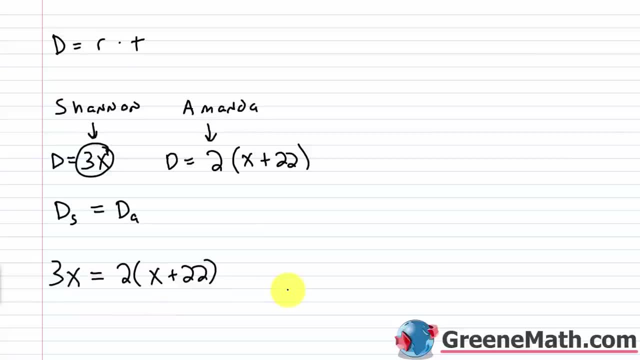 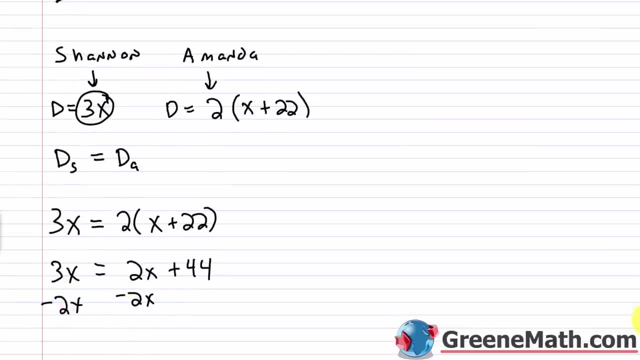 So, what I can do now is just solve this equation and find out rates of speed. So, over here, I'm going to simplify. 2 times x is 2x, plus 2 times 22, that's 44. Over here, I have 3x. Subtract 2x away from each side, very, very simple equation. We end up with x 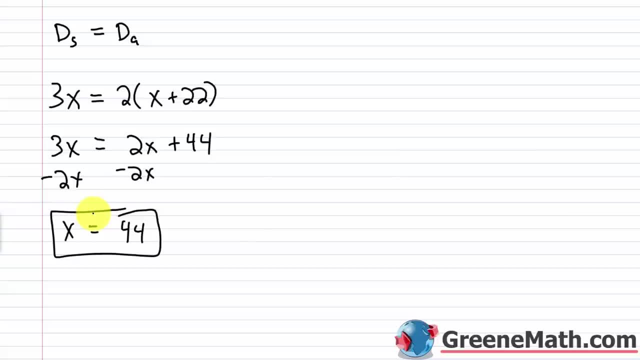 is equal to 44. Remember, 44 was the rate of speed for Shannon. Let x equal Shannon's speed in miles per hour. 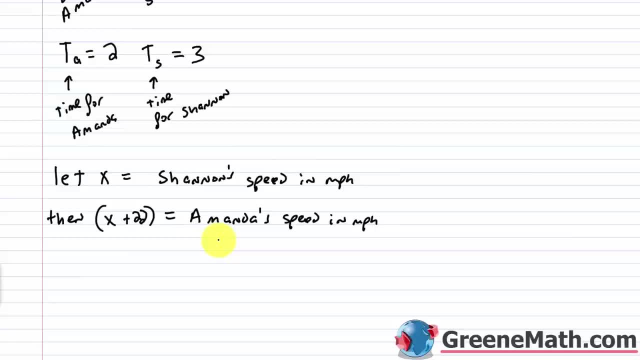 Then, x plus 22, or 44 plus 22, or 66, is Amanda's speed in miles per hour. 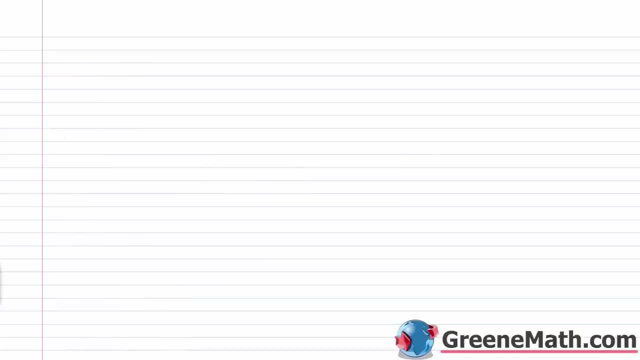 So, let's go ahead and write our answer. So, what was Shannon's average speed is our official question. average speed 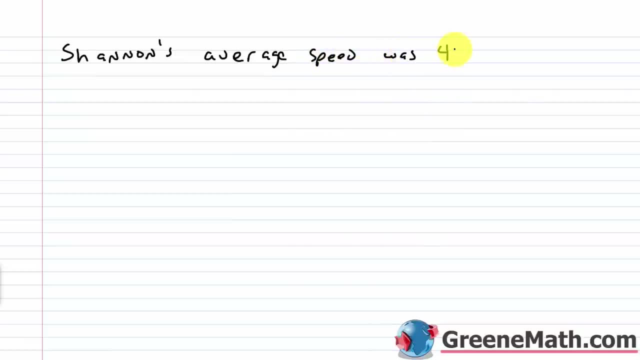 was 44 miles per hour. And we can check this to make sure that it's true. 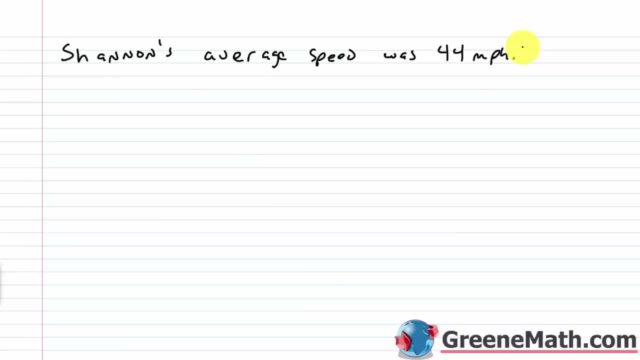 So, we know that Shannon traveled for 3 hours. So, 3 hours, think about your road trip. 3 hours times 44 miles per hour, how far am I going to go? I'm going to go 132 miles. 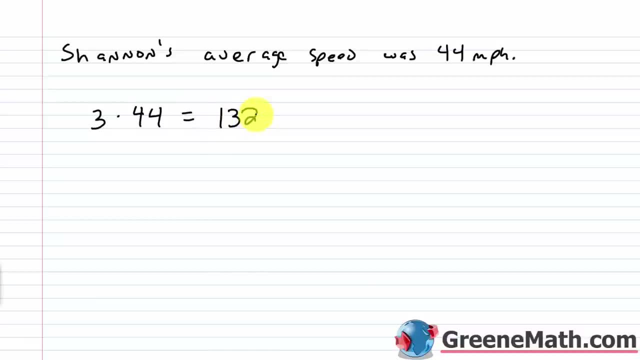 Now, we also know that Amanda leaves an hour after her. So, she only travels for 2 hours. She's traveling at x plus 22 miles per hour. x was 44. 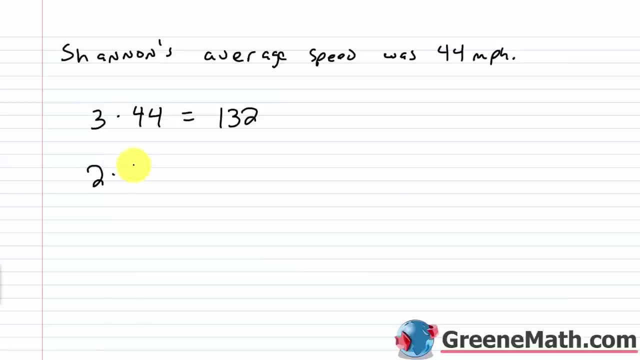 44 plus 22 is 66. So, 2 times 66. She drives for 2 hours at 66 miles per hour. 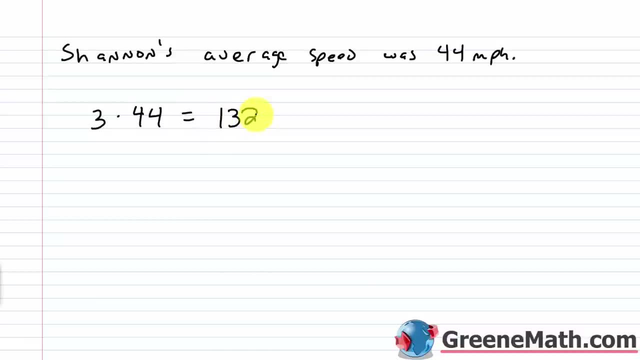 Now we also know that Amanda leaves an hour after her, So she only travels for two hours. She's traveling at X plus 22 miles per hour. X was 44.. 44 plus 22 is 66.. So two times 66.. 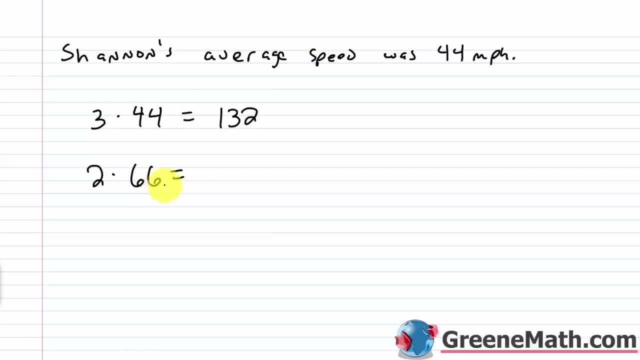 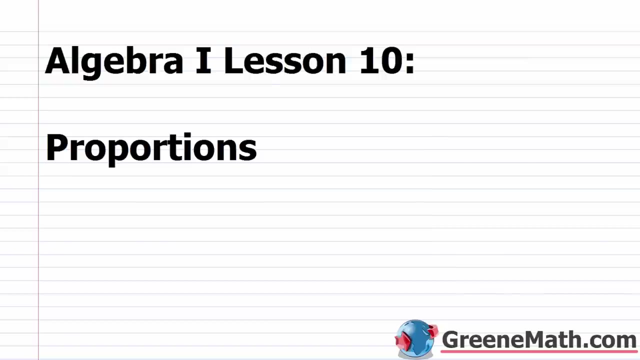 She drives for two hours at 66 miles per hour. How far does she go? She goes 132 miles, All right. So these distances again are equal And so we know we have the correct answer. Shannon's average speed here was 44 miles per hour. Hello and welcome to Algebra 1, Lesson 10.. 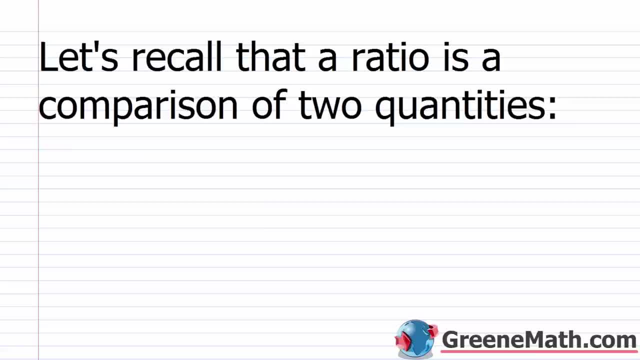 In this video we're going to learn about proportions. So before we get into proportions, let's recall that a ratio is a comparison of two quantities. So one way you might see this written: let's say you had the ratio of A to B. 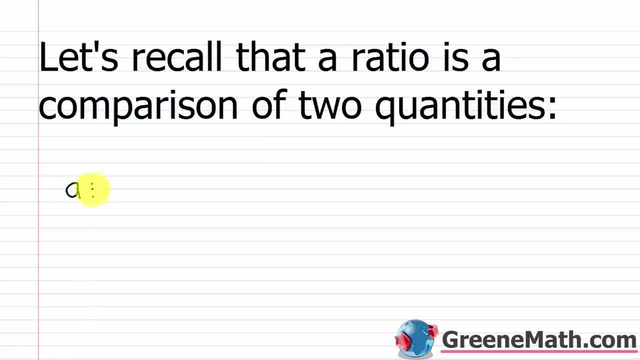 You might see it written with a colon, So you might see A and then a colon and then B. So this is the ratio of A to B. You also might see it written with the word two, So you might see A to B. And then, lastly, you might see it written as a fraction, So you might see A over B. 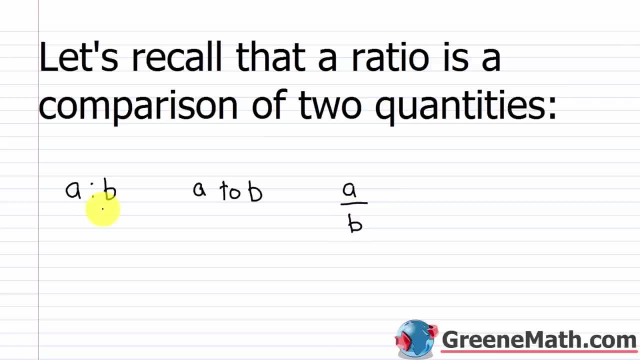 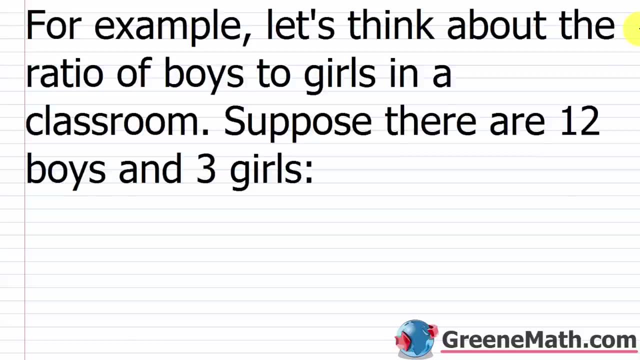 So each of these would be a different method to display the ratio A to B. All right, So as a quick example, let's think about the ratio of boys to girls in a classroom. So suppose there are 12 boys and three girls. So the ratio of boys to girls, 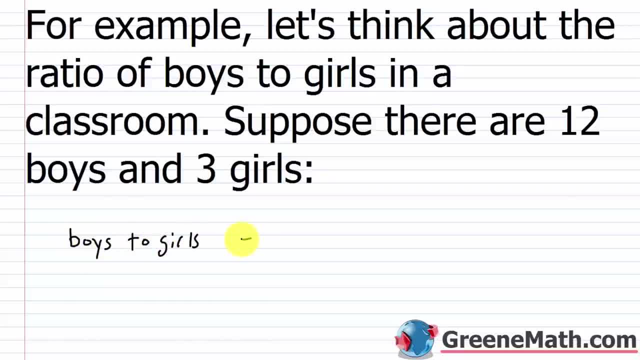 looks like this: You have 12 boys, 12 boys and you have three girls, So you can put 12 to three, like that, Or you could put 12 colon three, like that, Or you could put 12 over three. Now remember. 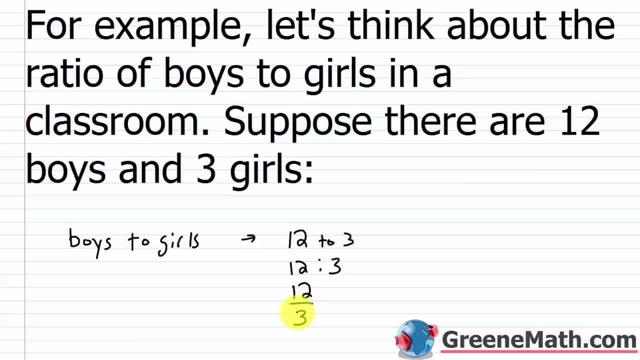 a ratio can be reduced to its lowest terms, the same way you would reduce a fraction. So you look at kind of the first part, the part that would be in the numerator, and you look at the last part, the part that would be in the denominator, and you say: hey, what's? 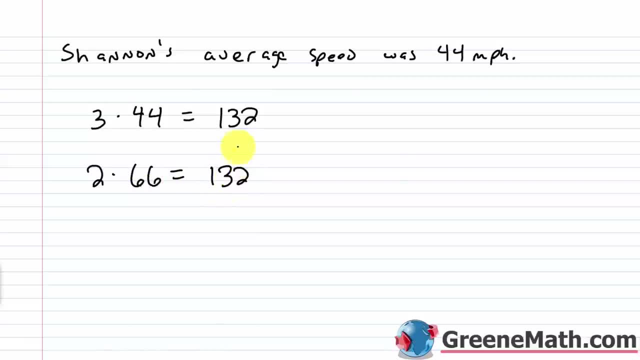 How far does she go? She goes 132 miles. Alright, so these distances again are equal. And so, we know we have the correct answer. Shannon's average speed here was 44 miles 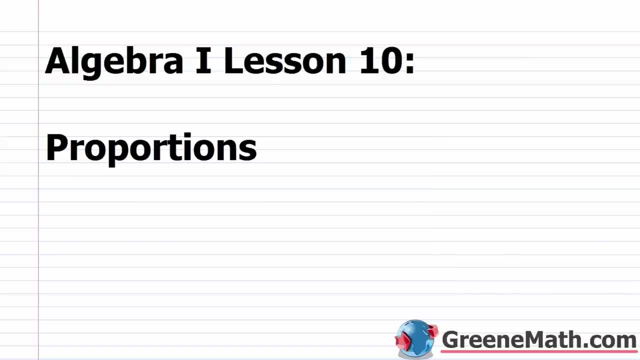 per hour. Hello, and welcome to the Algebra 1 Lesson 10. 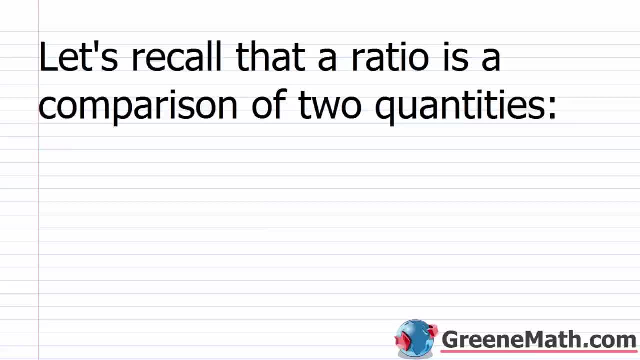 In this video, we're going to learn about proportions. So, before we get into proportions, let's recall that a ratio is a comparison of two quantities. So, one way you might see this written, let's say you had the ratio of A to B. You might see it written with a colon. So, you might see A and then a colon and then B. So, this is the ratio of A to B. You also might see it written with the 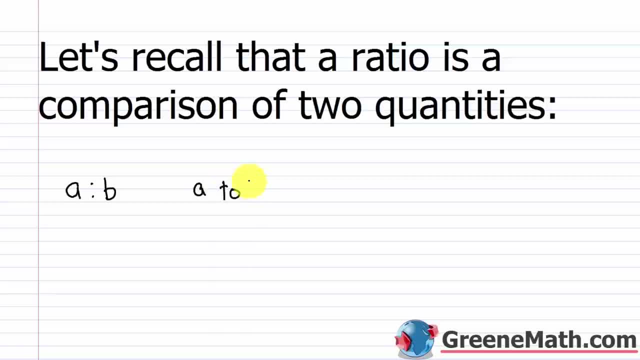 word 2. So, you might see A to B. 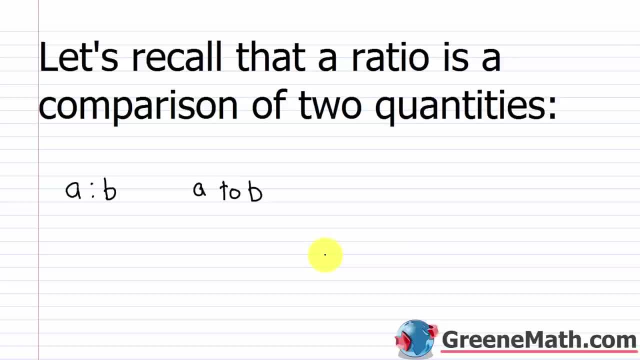 And then, lastly, you might see it written as 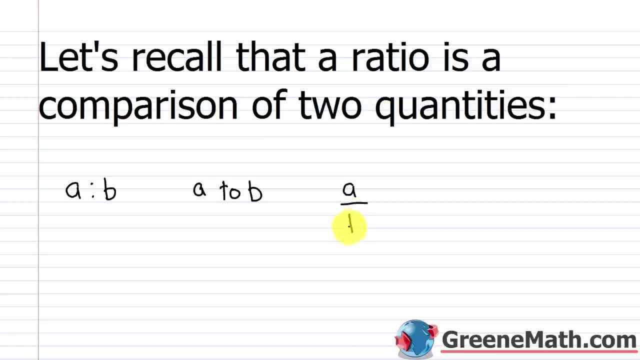 a fraction. So, you might see A over B. 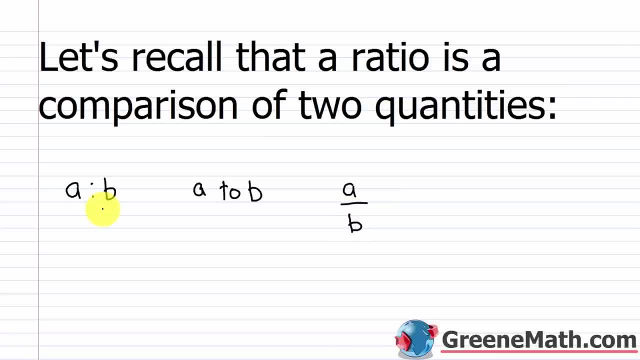 So, each of these would be a different method to display the ratio A to B. 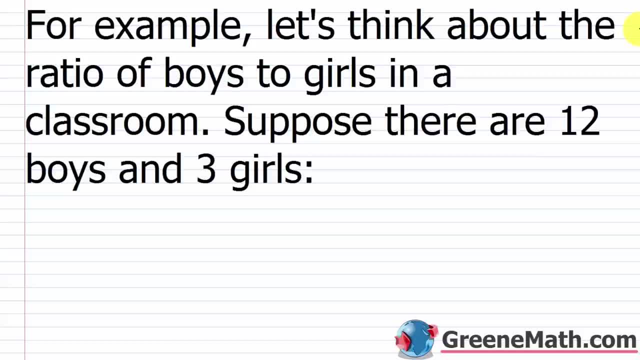 Alright, so as a quick example, let's think about the ratio of boys to girls in a classroom. So, suppose there are 12 boys and 3 girls. So, the ratio of boys to girls looks like this. You have 12 boys 12 boys and you have 3 girls. 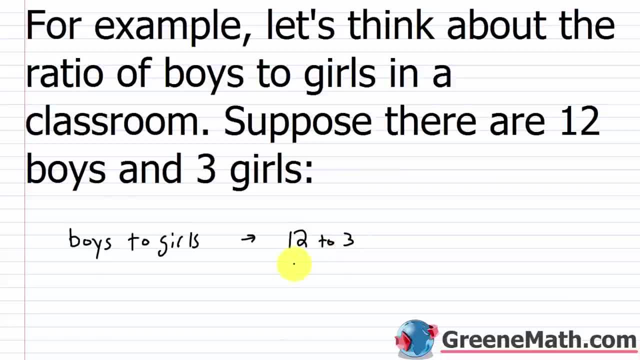 So, you can put 12 to 3 like that. 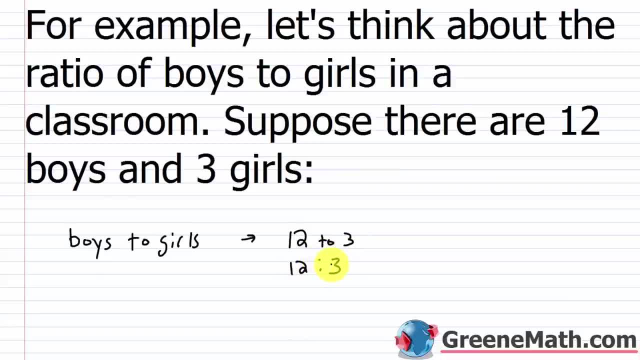 You could put 12 colon 3 like that. 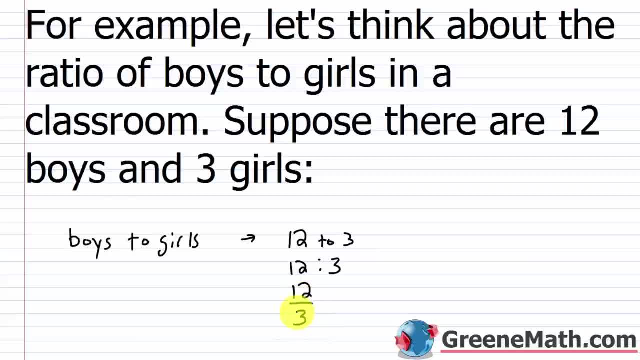 Or, you could put 12 over 3. 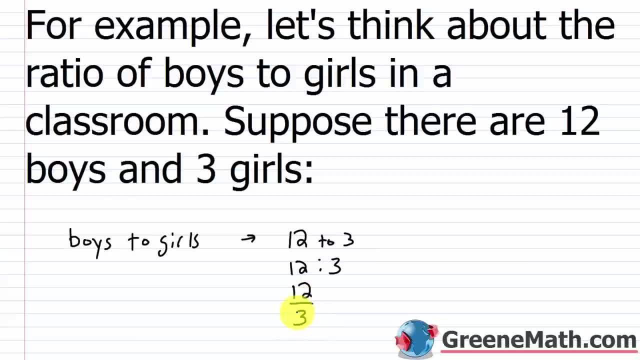 Now, remember a ratio can be reduced to its lowest terms. The same way you would reduce a fraction. 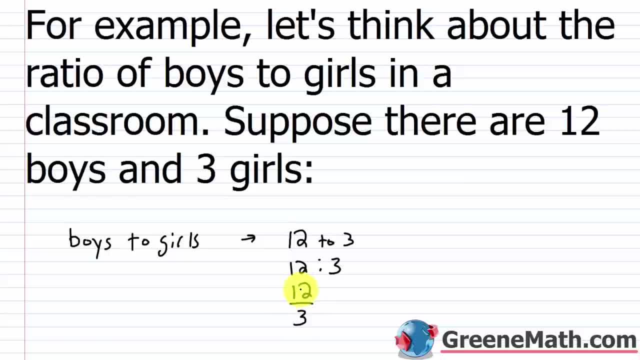 So, you look at kind of the first part, the part that would be in the numerator and you look at the last part, the part that would be in the denominator and you say, hey, what's my greatest common factor? 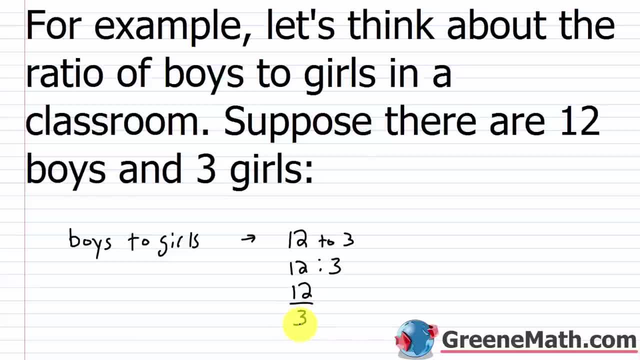 my greatest common factor. So when we look at 12, and we look at three, the GCF would be three. So if I divide 12 by three, I get four. If I divide three by three, I get one. So the 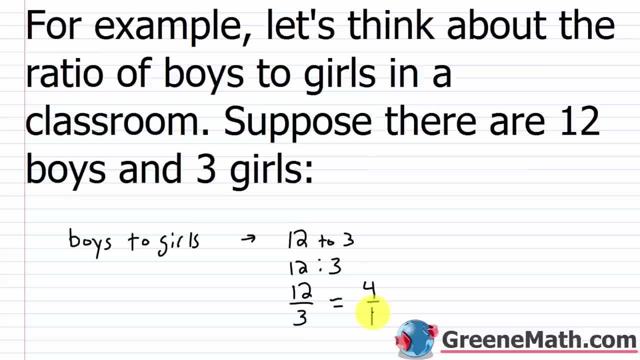 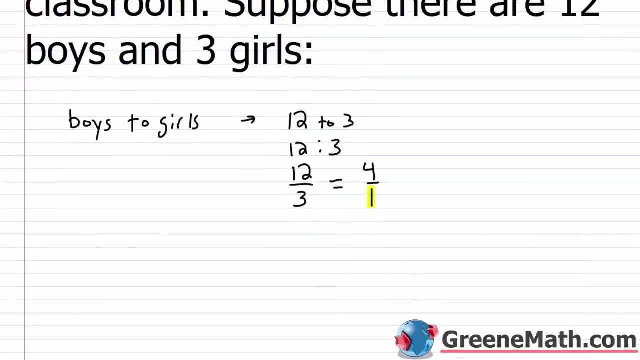 ratio of 12 to three can be simplified and thought of as the ratio of four to one. Now, a lot of times I know when working with fractions we might get rid of this one. We might just write that as the number four. When we're working with ratios we don't do that. So 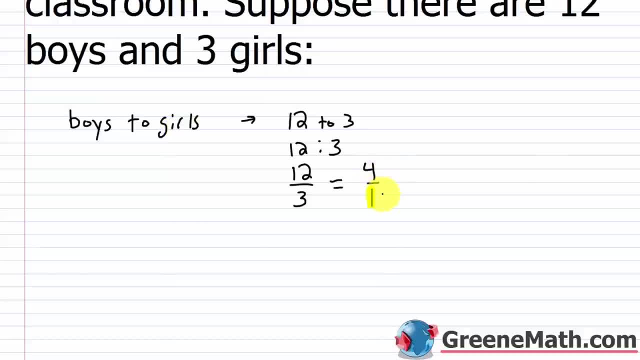 if I have the ratio of boys to girls, I want to say it's four to one. I don't want to just say it's four, right, So you want that one there. It's very important when you're working with a ratio to just leave it there, because you're talking about a comparison. 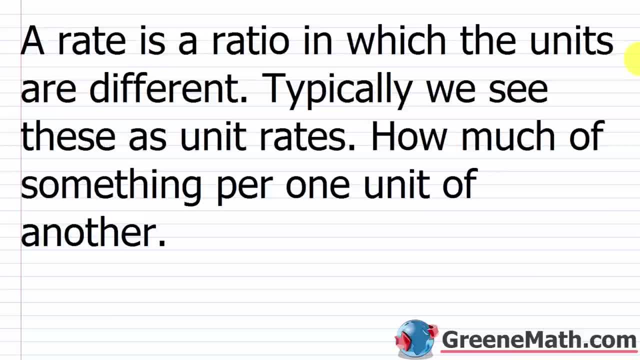 of one thing to another. All right, let's talk a little bit about a rate. So a rate is also a ratio, and this is one in which the units are different. So the units are different. So typically we see these as unit rates. okay, Unit rates. And every time you go into a grocery store, 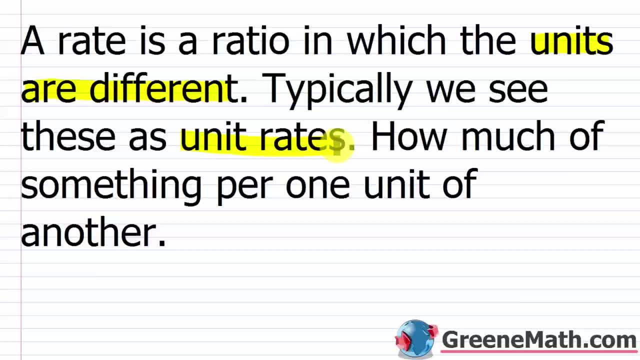 you're going to deal with this. If you look at the little grocery labels next to the price, it'll probably say this is the price per ounce, or this is the price per pound, you know so on and so forth. So how much of something per one unit of another? So you can think. 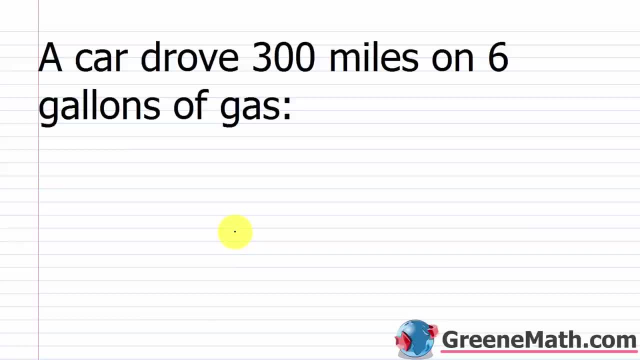 about. a car drove 300 miles on six gallons of gas. You can use this information to set up a unit rate and figure out the miles per gallon here. So 300 miles, 300 miles, put that in the numerator and then I'm going to put six gallons. 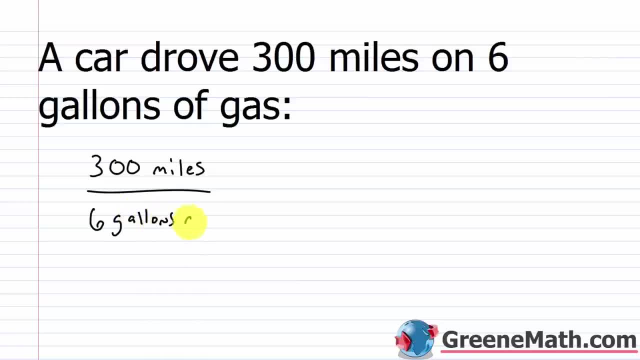 Six gallons of gas in the denominator. So we have 300 miles per. you can think of your fraction bar as saying per six gallons of gas, And we could simplify this by looking at the numbers. If I divide 300 by six, I would get 50.. So I would write 50, and the 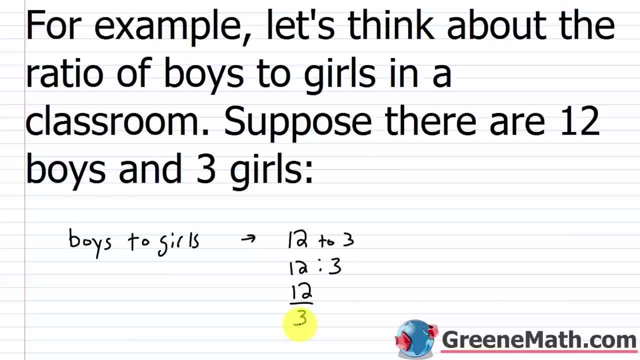 So, when we look at 12 and we look at 3, the GCF would be 3. So, if I divide 12 by 3, I get 4. 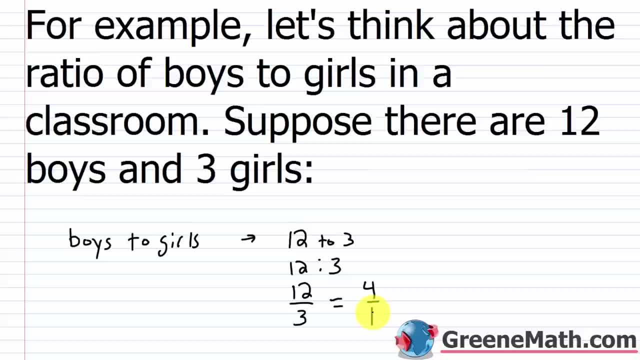 If I divide 3 by 3, I get 1. 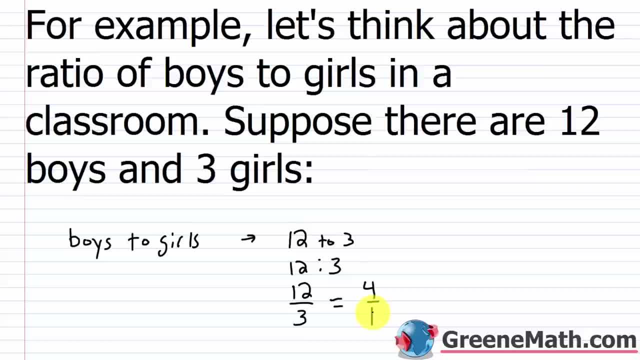 So, the ratio of 12 to 3 can be simplified and thought of as the ratio of 4 to 1. 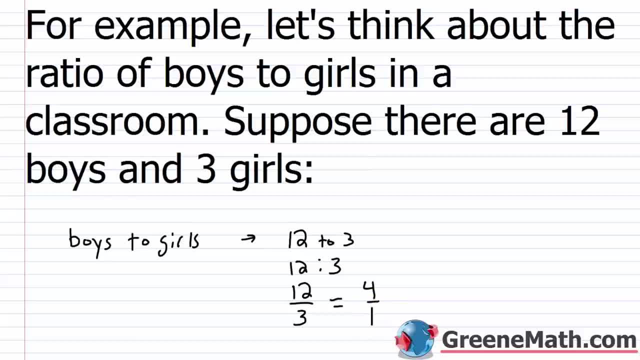 Now, a lot of times, I know when working with fractions, we might get rid of this 1. We might just write that as the number 4. 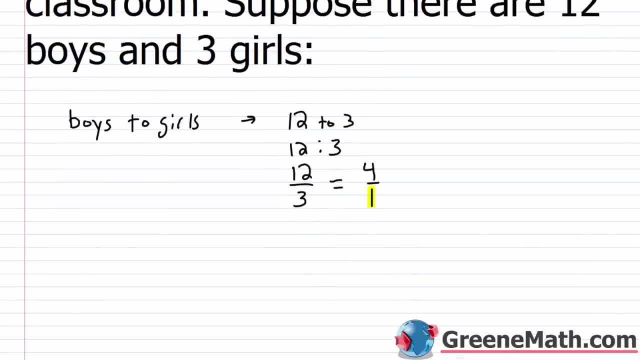 When we're working with ratios, we don't do that. So, if I have the ratio of boys to girls, I want to say it's 4 to 1. I don't want to just say it's 4. So, you want that 1 there. It's very important when you're working with a ratio to just leave it there because you're talking about a comparison of one thing to another. 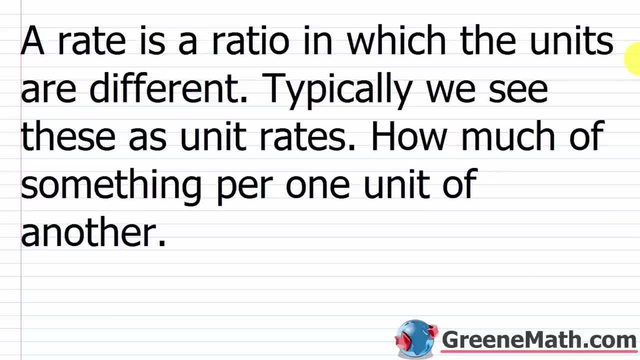 Alright, let's talk a little bit about a rate. So, a rate is also a ratio and this is one in which the units are different. So, the units are different. So, typically we see these as unit rates. Unit rates. And every time you go into a grocery store, you're going to deal with this. If you look at the little grocery labels next to the price, it'll probably say this is the price per ounce or this is the price per pound. You know, so on and so forth. 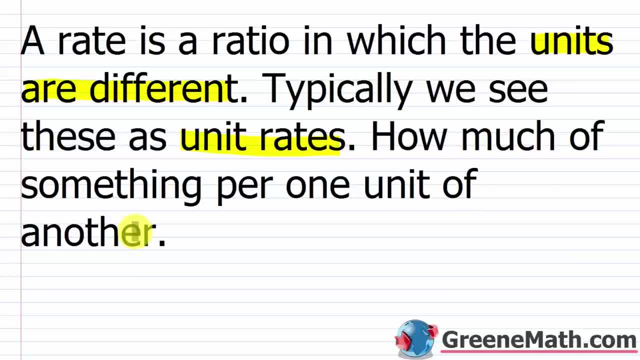 So, how much of something per one unit of another. 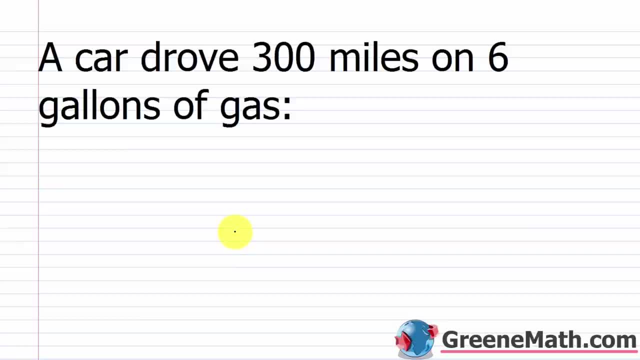 So, you can think about a car drove 300 miles on 6 gallons of gas. You can use this information to set up a unit rate and figure out the miles per gallon here. So, 300 miles, 300 miles. 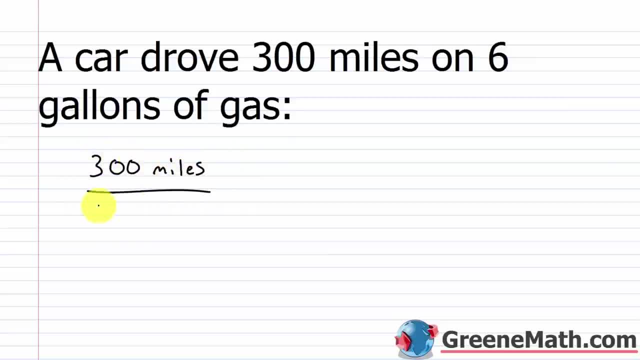 Put that in the numerator and then I'm going to put 6 gallons 6 gallons of gas in the denominator. 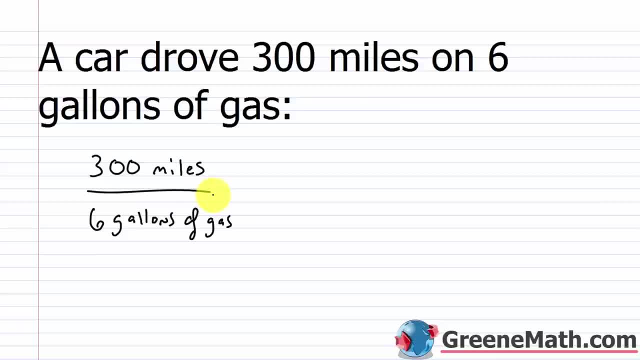 So, we have 300 miles per, you can think of your fraction bar as saying per, 6 gallons of gas. 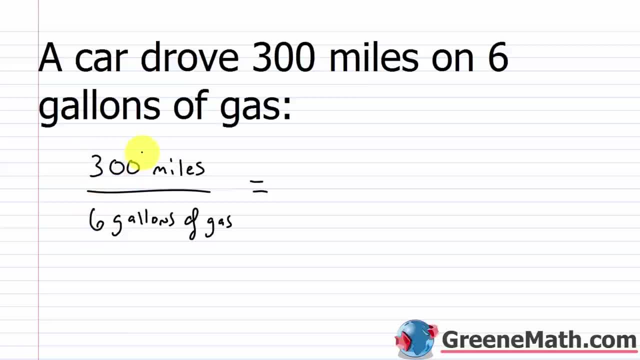 And we can simplify this by looking at the numbers. If I divide 300 by 6, I would get 50. So, I would write 50 and the units are going to stay there. 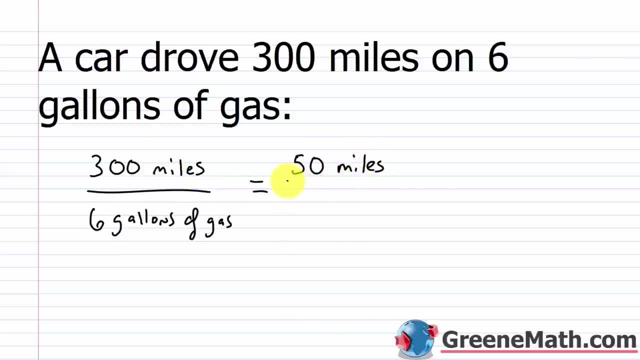 units are going to stay there: Miles per. and then if I divide six by six, I'm going to get one. So one gallon of gas, So 50 miles per one gallon of gas, And that's very, very common. We're always thinking about our fuel economy, So what is the number of miles I'm 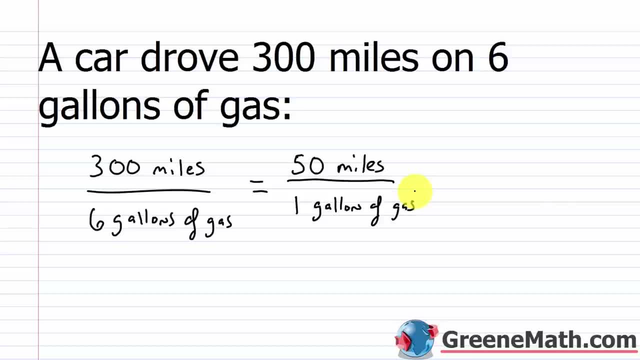 going to get per gallon of gas, you know on average. So if you do a road trip, you can track how many miles you do and on how many gallons of gas, and you can set up the same thing. You could figure out your miles per gallon. And one thing about a unit rate: 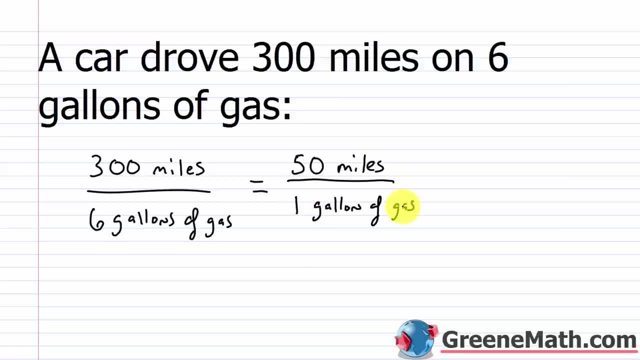 notice that the units do not cancel. So with a typical ratio we have the same units and so we really don't list them right. You don't need to, because you could think of them as kind of canceling out. Here I have miles in the numerator and I have gallons of gas. 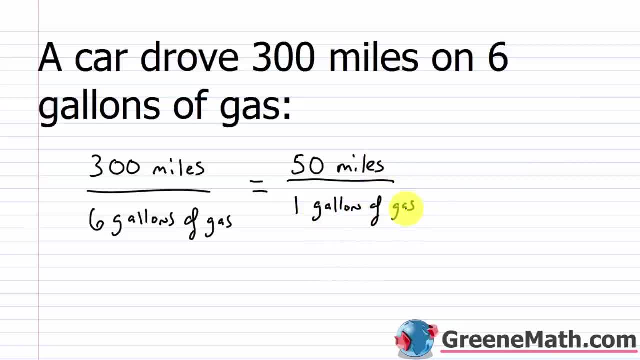 or gallon of gas in the denominator. So those we're going to write right for clarity. They don't cancel out, so we just keep them there And basically the only thing you need to understand is you're always going to take the number in the numerator, which, in this, 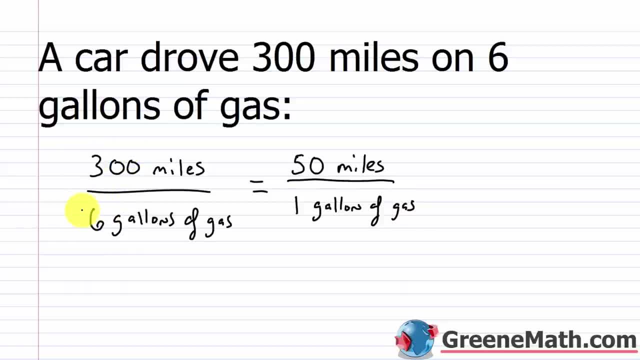 case is 300, and divide it by the number And the denominator, which there is 6.. That's going to give you some amount in the numerator per one amount in the denominator. So it's always per a single unit. You always want. 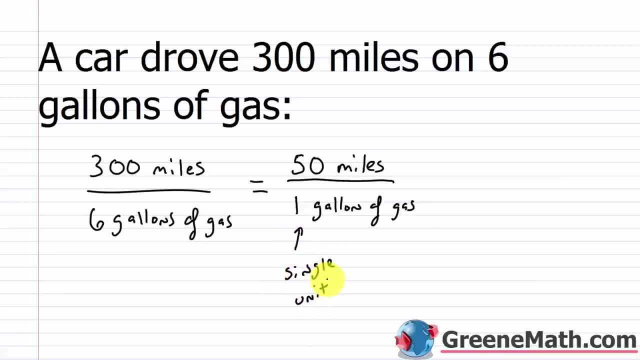 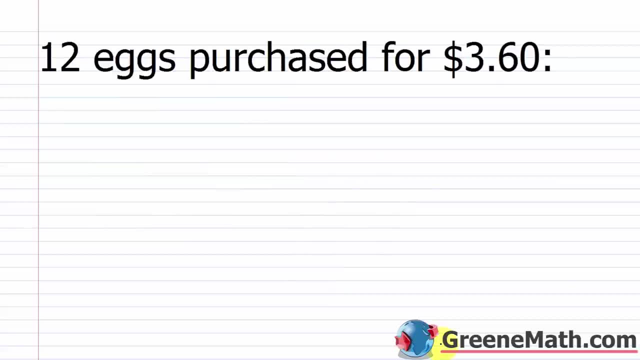 a single unit in the denominator. That's why it's called a unit rate. So let's take a look at another one real quick. So 12 eggs purchased for $3.60. So I can put $3.60 in the numerator. 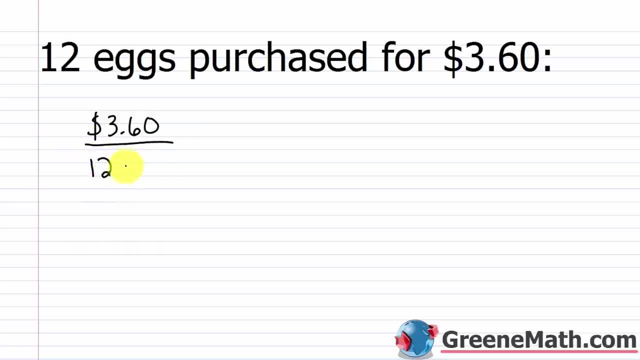 and I can put per 12 eggs in the denominator, And what I'll do is I'll divide this $3.60, or just 3.60, by 12, and I'm going to get a unit rate which is a cost per one egg. 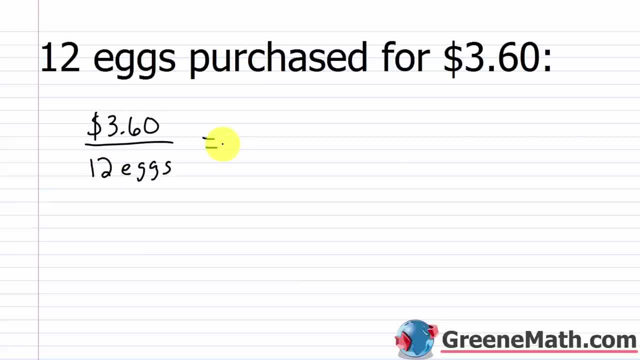 So if I divide 3.60 by 12, I get 0.3.. So I would get $0.3 per one egg, right? So I'm going to do that. So this is the unit cost, right, The cost per one egg. And again, I. 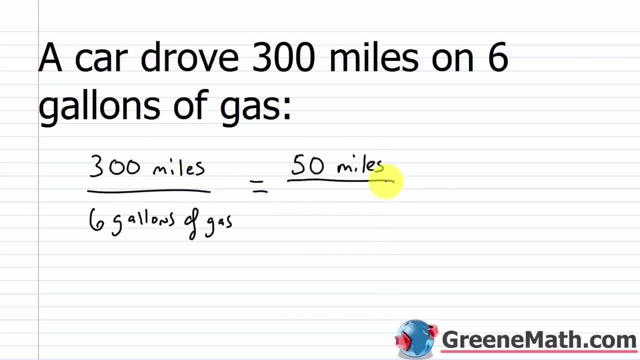 Miles per, and then if I divide 6 by 6, I'm going to get 1. So, 1 gallon of gas. So, 50 miles per 1 gallon of gas. And that's very, very common. We're always thinking about our fuel economy. So, what is the number of miles I'm going to get per gallon of gas on average? So, if you do a road trip, you can 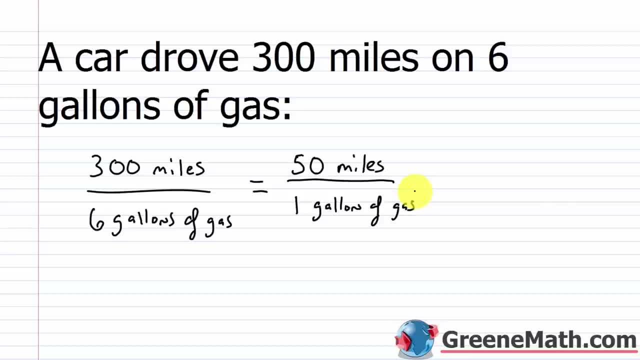 track how many miles you do and on how many gallons of gas 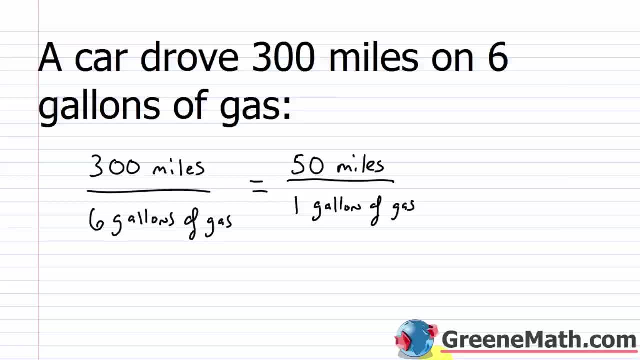 and you can set up the same thing. You can figure out your miles per gallon. And one thing about a unit rate, you're going to notice that the units do not cancel. So, with a typical ratio, we have the same units and so we really don't list them. You don't need to because you can think of them as kind of canceling out. Here, I have miles in the numerator and I have gallons of gas or gallon of gas in the denominator. So, those we're going to write for clarity. 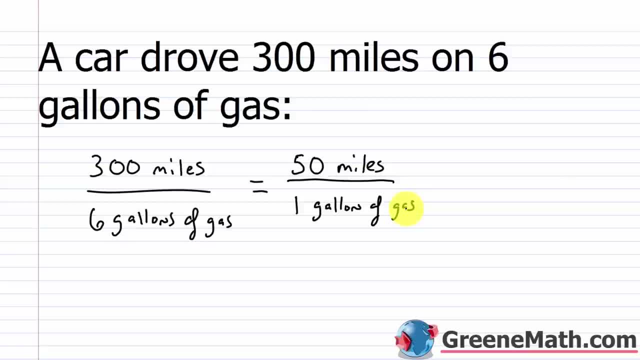 They don't cancel out, so we just keep them there. And basically, the only thing you need to understand is you're always going to take the number in the numerator, which in this case is 300, and divide it by the number in the denominator, which there is 6. That's going to give you some amount in the numerator per 1 amount in the denominator. So, it's always per a single unit. 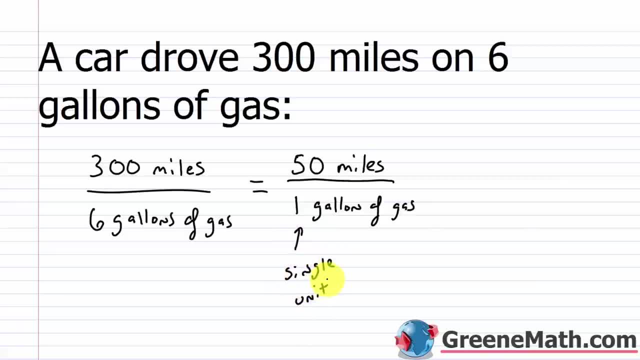 You always want a single unit in the denominator. 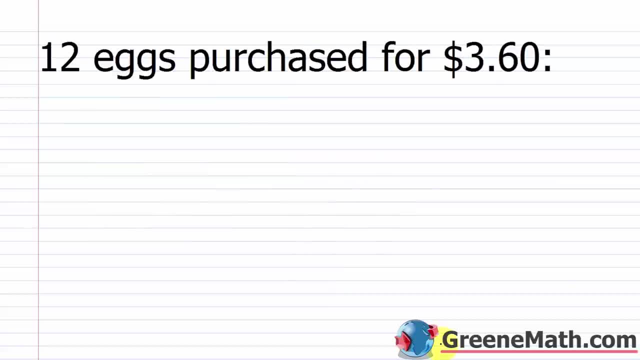 That's why it's called a unit rate. Let's take a look at another one real quick. 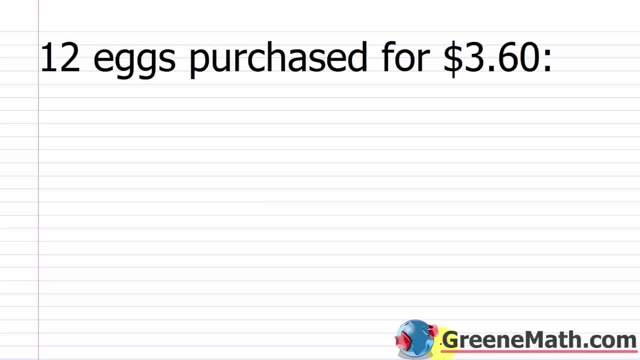 So, 12 eggs purchased for $3.60. So, I can put $3.60 in the numerator and I can put per 12 eggs in the denominator. 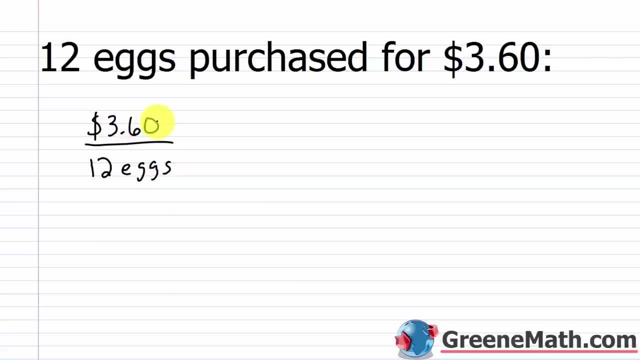 And what I'll do is I'll divide this $3.60 or just 3.60 by 12 and I'm going to get a unit rate, which is a cost per 1 egg. So, if I divide 3.60 by 12 I get .3. So, I would get .3 dollars per 1 egg. 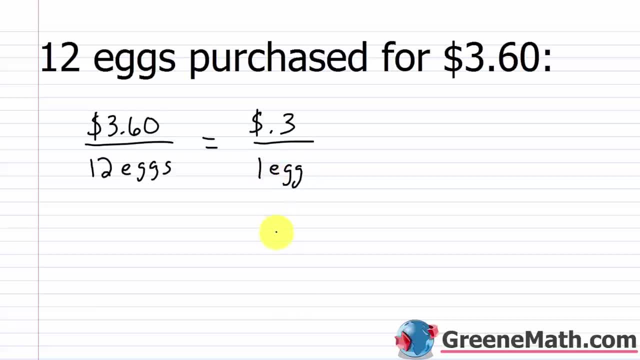 So, this is the unit cost. The cost per 1 egg. And again, I take the number part from the numerator and I divide it by the number part in the denominator, and that's going to give me my unit cost. So, this denominator will always be singular. So, instead of eggs, it becomes egg. And then the numerator, whatever number you end up with, it's going to be the value per 1 unit. 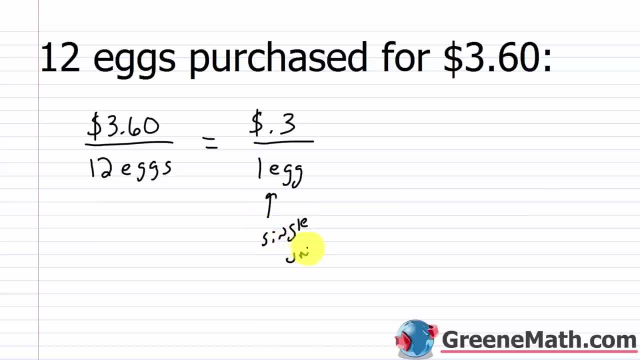 So, again, this is a single unit. 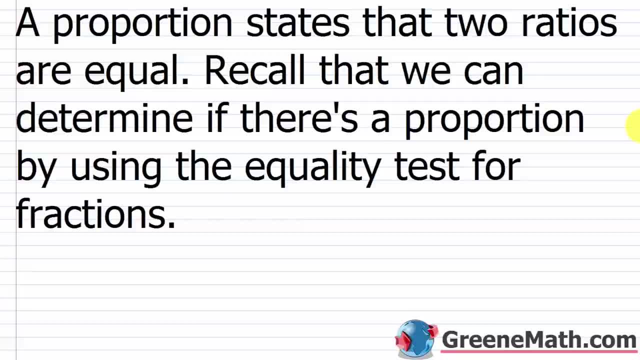 Alright, so now that we've kind of reviewed the basics of what a ratio 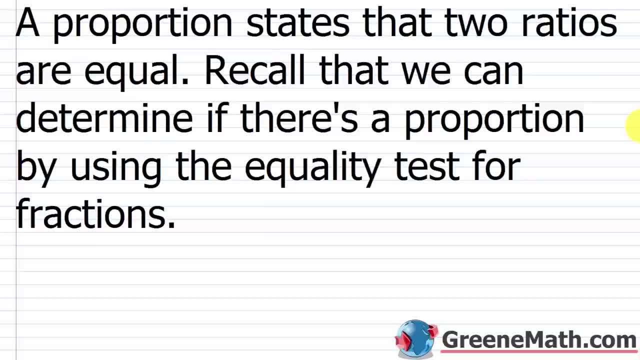 is, let's talk a little bit about a proportion. So, we talked about this in 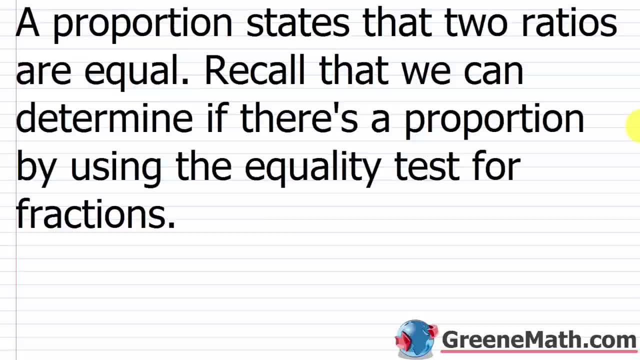 pre-algebra. A proportion states that two ratios are equal. 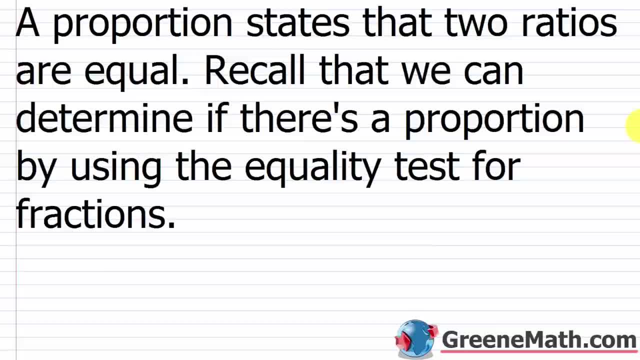 And a lot of times, we're just looking at two fractions. We're trying to see if those two fractions are equal. And if they are, we say that we have a proportion. So, I want you to recall 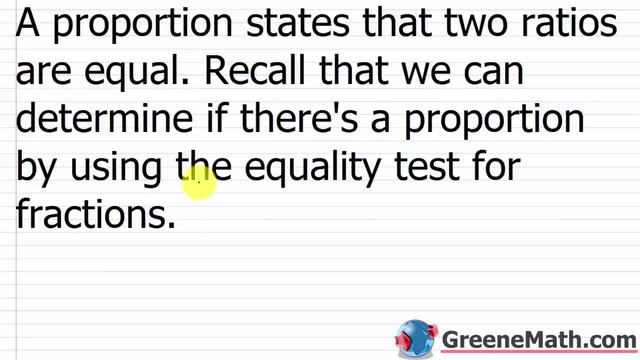 that we can determine if there's a proportion by using the equality test for fractions. The equality test for fractions. 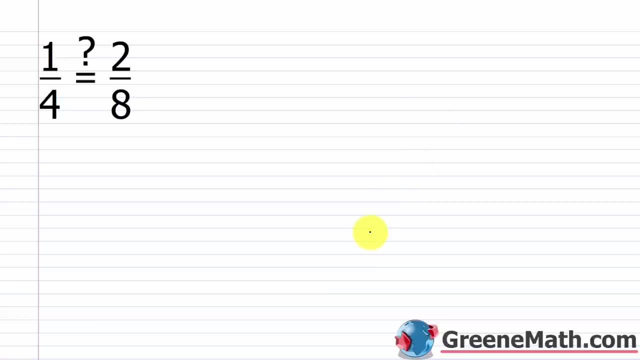 How do we do the equality test for fractions? It's very, very simple. I take the denominator of one fraction, and I multiply it by the numerator of the other. So, 4 times 2 is 8. And I look at that value. I then take the denominator of the other fraction, and I multiply it by the numerator of the other fraction. 8 times 1 is 8. 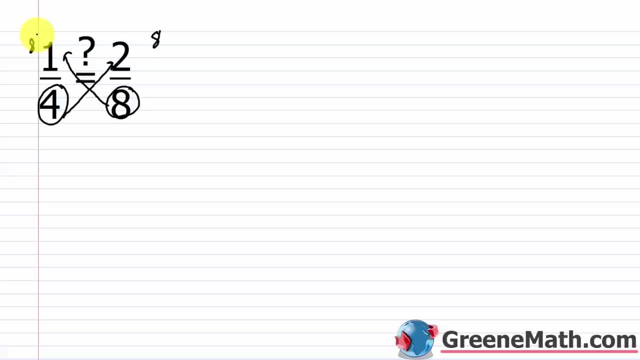 If I get the same value on each side, then the fractions are equal, or you could say the ratios are equal, however you want to think about it. 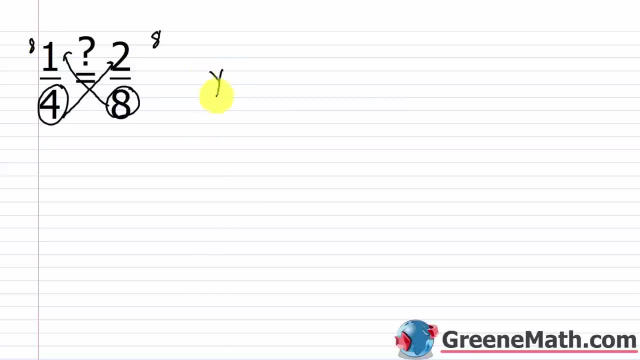 And so, you have a proportion. So, yes, this is a proportion. 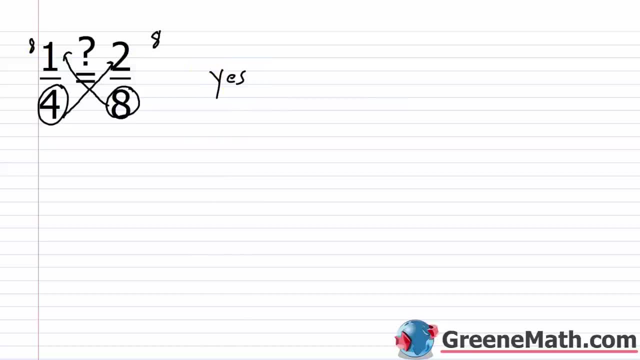 And it's important to note that this is called cross multiplying. So, it's always going to be the denominator of your first fraction times the numerator of the second one. 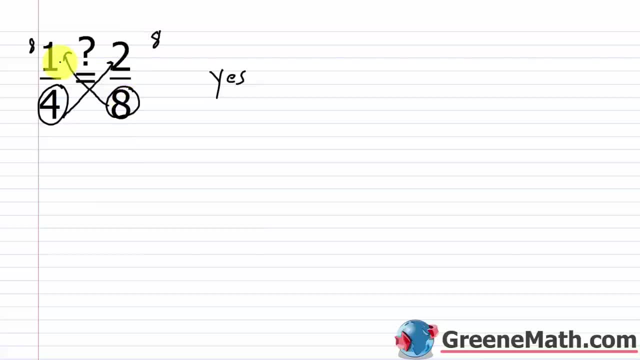 And then, the denominator of the second one times the numerator of the first one. 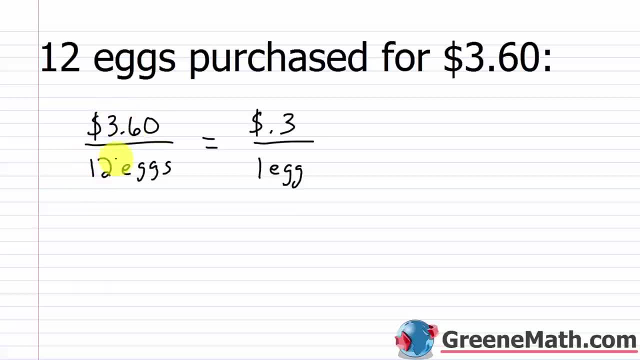 take the number part from the numerator and I divide it by the number part in the denominator and that's going to give me my unit cost. So this denominator will always be singular. So instead of eggs it becomes egg. And then the numerator, whatever number you end up. 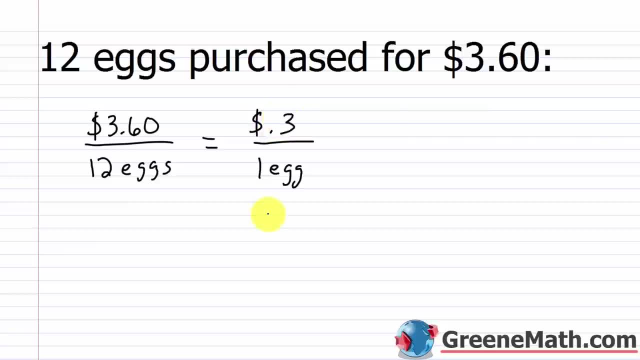 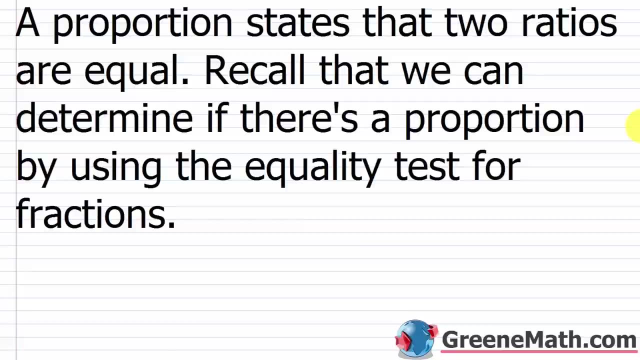 with, it's going to be the value per one unit. So again, this is a single unit And that's why we call it a unit rate. All right, So now that we've kind of reviewed the numerator and denominator, we're going to go ahead and 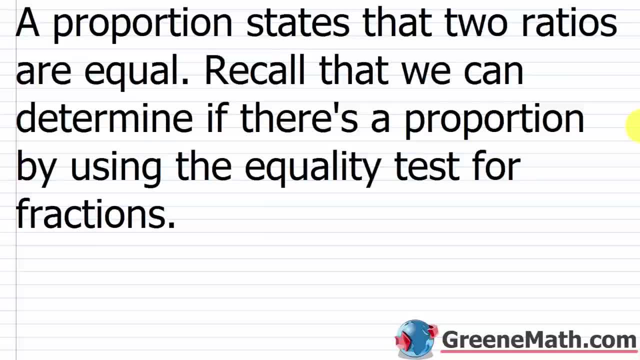 look at the basics of what a ratio is. Let's talk a little bit about a proportion. So we talked about this in pre-algebra. A proportion states that two ratios are equal And a lot of times we're just looking at two fractions, right, And we're trying to see if those two 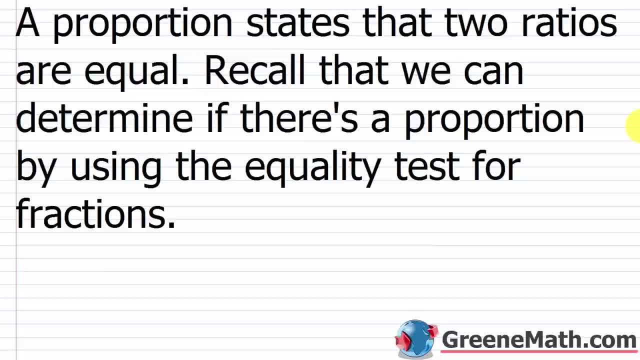 fractions are equal And if they are, we say that we have a proportion. So I want you to recall that we can determine if there's a proportion by using the equality test for fractions, The equality test for fractions. How do we do the equality test? 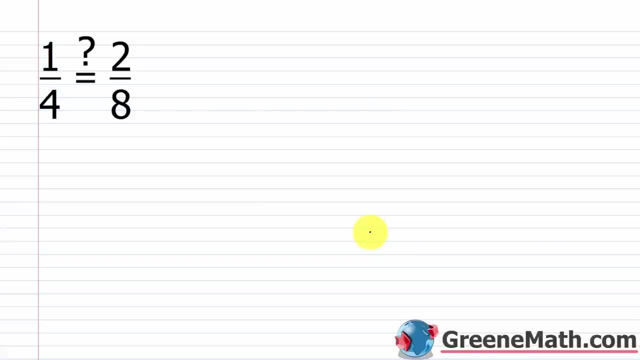 for fractions. It's very, very simple. I take the denominator of one fraction and I multiply it by the numerator of the other. So four times two is eight, And I look at that value. I then take the denominator of the other fraction and I multiply it by the numerator of the other fraction. 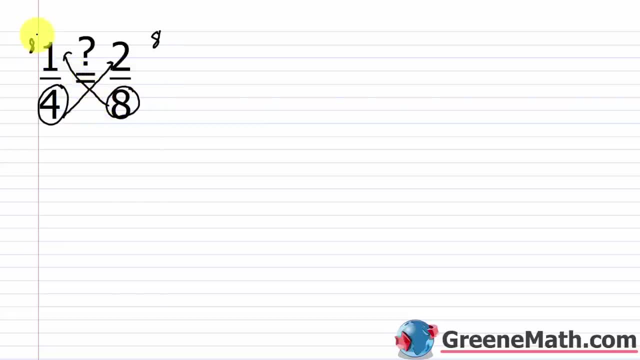 Eight times one is eight. If I get the same value on each side, then the fractions are equal, or you could say the ratios are equal, however you want to think about it, And so you have a proportion. So, yes, this is a proportion, And it's important to note that. 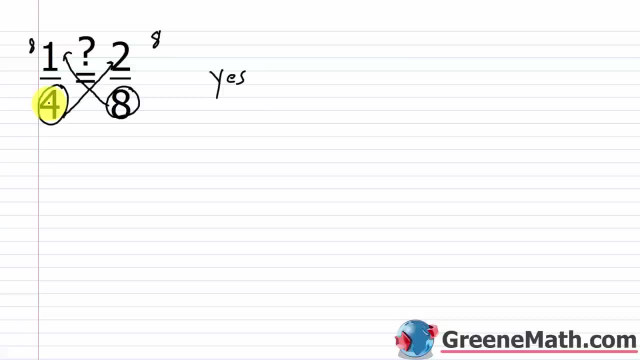 this is called cross-multiply, So it's always going to be the denominator of your first fraction times the numerator of the second one, And then the denominator of the second one times the numerator of the first one. Let's take a look at this one. We have three-eighths and four-sevenths. We want to know if we have. 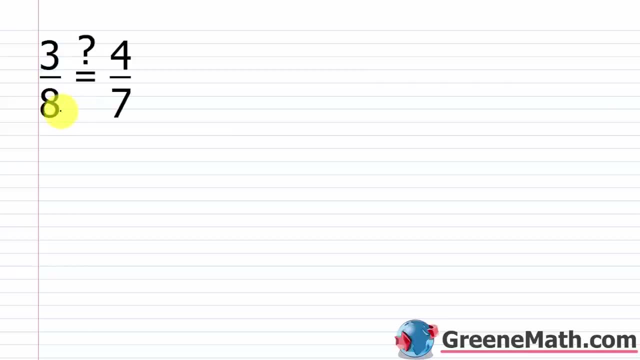 a proportion. So again we're going to cross-multiply. So I would take the denominator of this fraction here, multiply it by the numerator of this fraction here. Eight times four is thirty-two. Then I'd take the denominator of this fraction here. 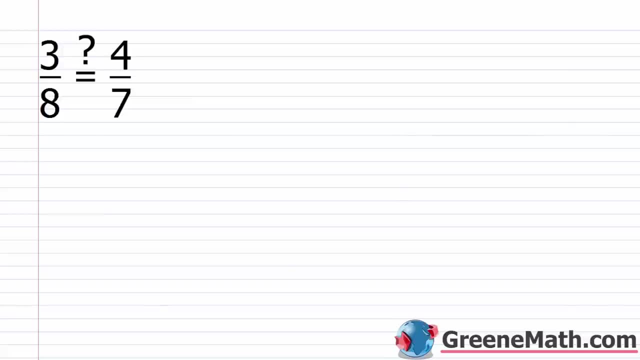 Let's take a look at this one. We have 3 eighths and 4 sevenths. We want to know if we have a proportion. So, again, we're going to cross multiply. So, I would take the denominator of this fraction here, multiply it by the numerator of this fraction here. So, 8 times 4 is 32. 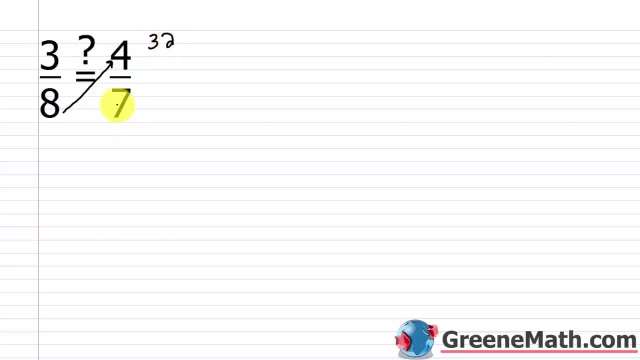 Then, I take the denominator of this fraction here, and I multiply it by the numerator of this fraction here. 7 times 3 is 21. So, we do not have the same value. 21 is not the same as 32. So, this is no. It's not a proportion. Again, in order to have a proportion, 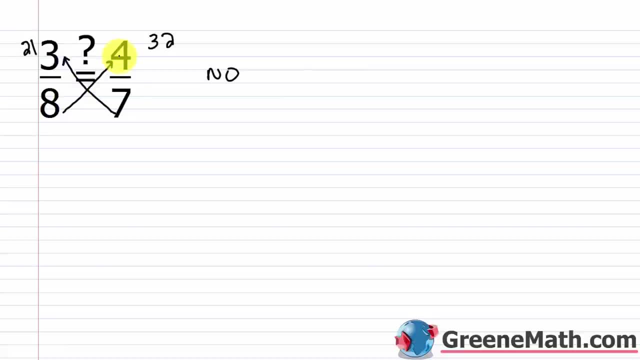 this times this has to be the same as this times this. You have to get the same 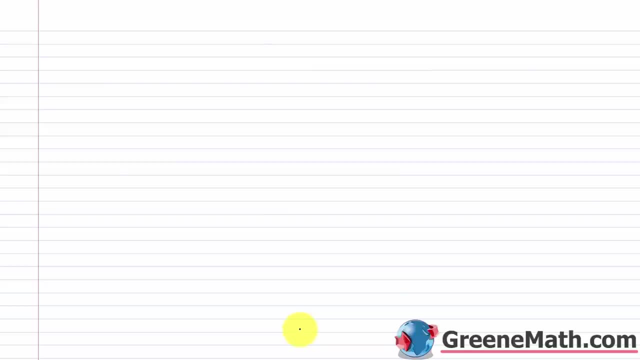 value. So, before we kind of move on to solving a proportion equation, 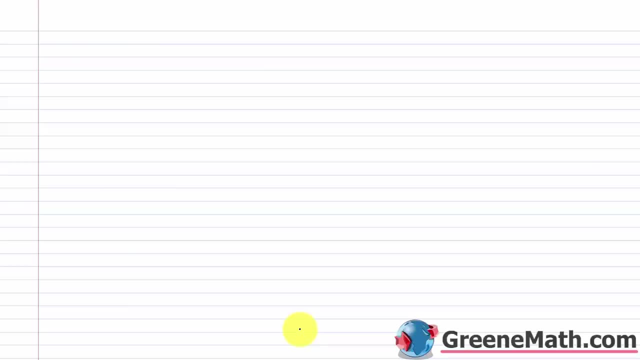 I want to kind of cover something you're going to see in your textbook. 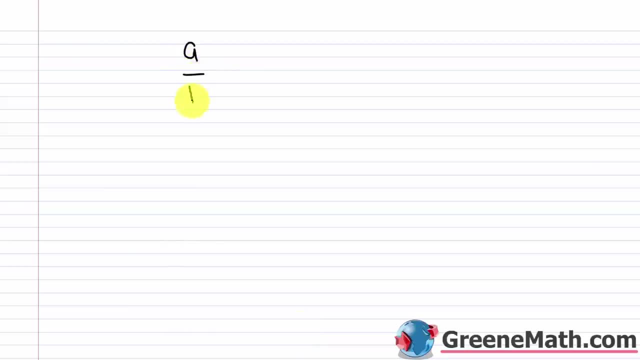 So, you're going to see that if A over B is equal to C over D, then it must be true that AD is equal to BC. 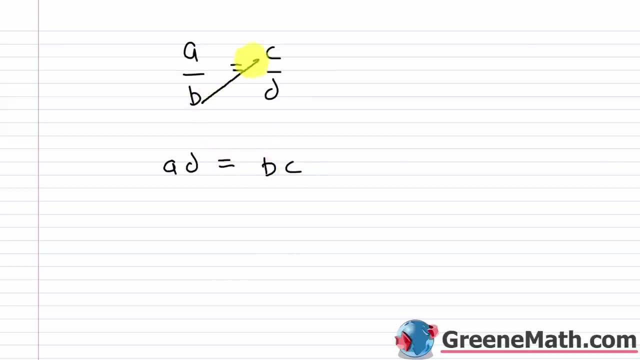 So, what they're doing is they're cross multiplying. They're saying, okay, B times C is BC. 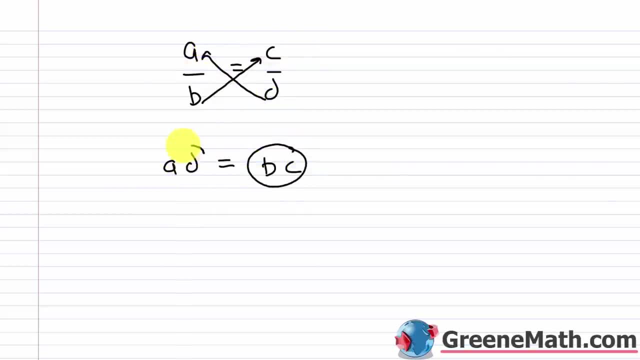 And that has to be equal to D times A, which is AD. Or DA, or however you want to write that. It doesn't matter. 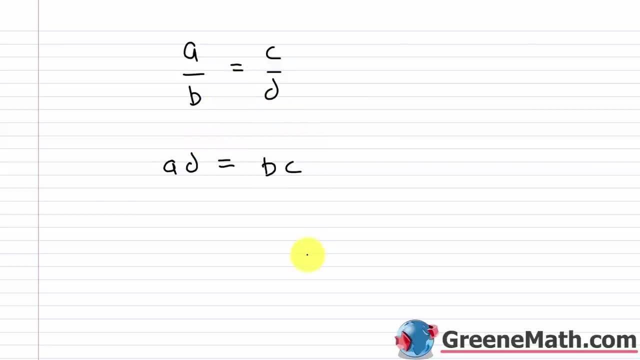 Now, you might think about, where did this cross multiplication come from? 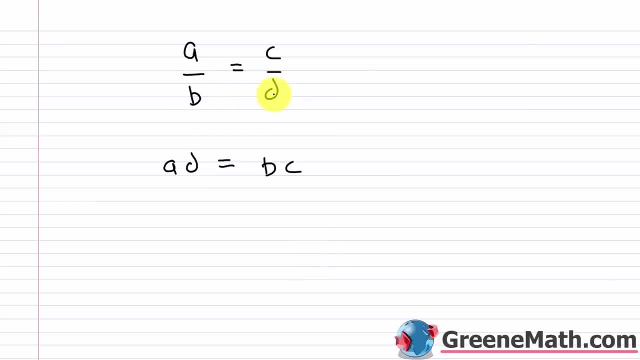 Well, if I kind of look at the denominators here, I have B and I have D. 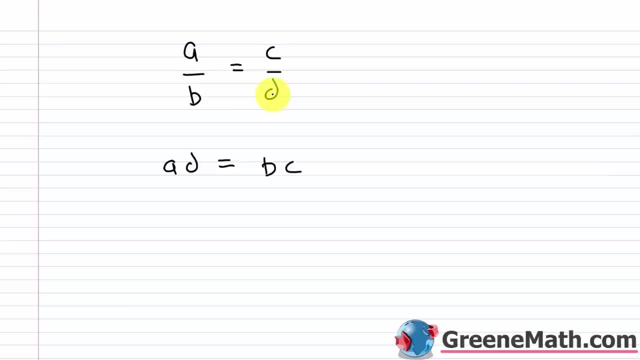 So, let's say I multiplied both sides of the equation by the LCD, which is BD. 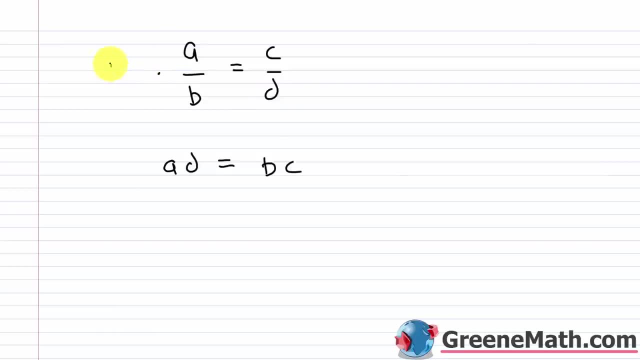 B times D. If I multiply this side by BD, which is perfectly legal with an equation, as long as I do it to this side, we see here that this would cancel here, and we also see that this would cancel here. So, what would I have left? I'd have D times A, which is the same as AD. I just switched the order. 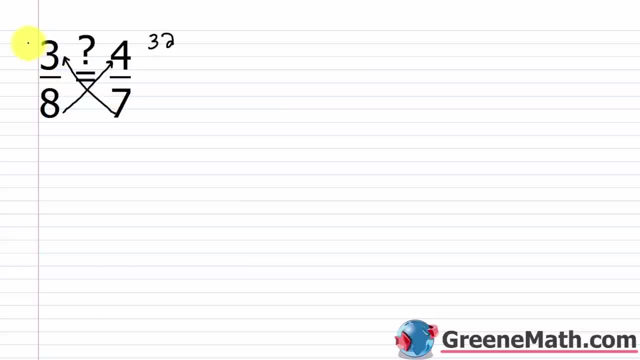 and I'd multiply it by the numerator of this fraction here. Seven times three is twenty-one, So we do not have the same value. Twenty-one is not the same as thirty-two, So this is no, It's not a proportion. Again, in order to have a proportion, this times this has: 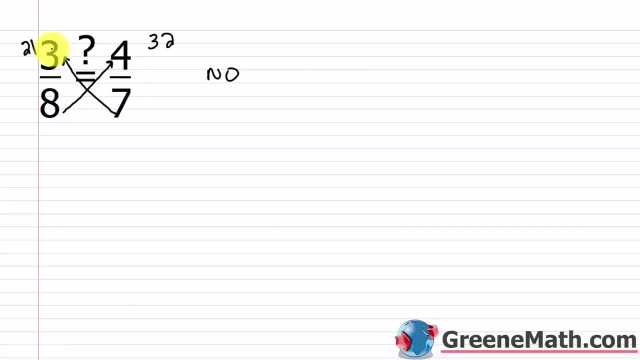 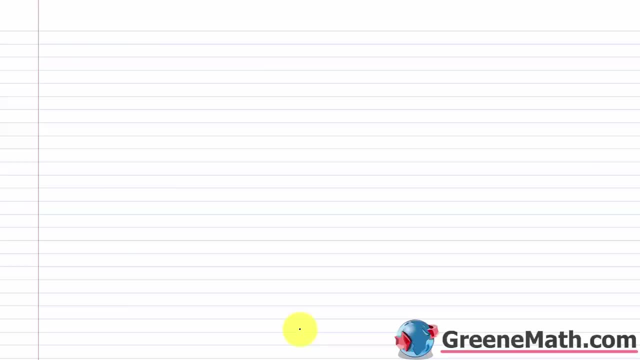 to be the same as this. times this Have to get the same value. So before we kind of move on to solving a proportion equation, I want to kind of cover textbook. So you're going to see that if a over b is equal to c over d, then it must. 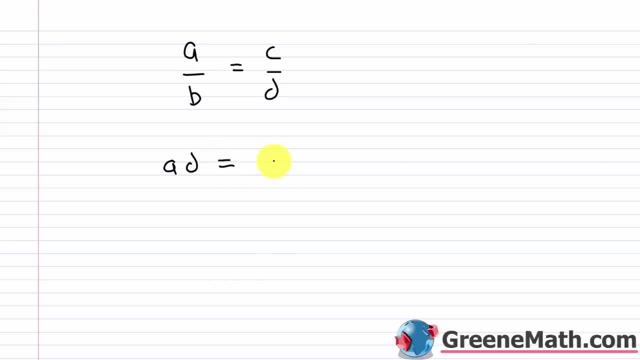 be true that ad is equal to bc. So what they're doing is they're cross-multiplying. They're saying, okay, b times c is bc, And that has to be equal to d times a, which is ad or da, or however you want to write that It doesn't matter. Now you might think about. 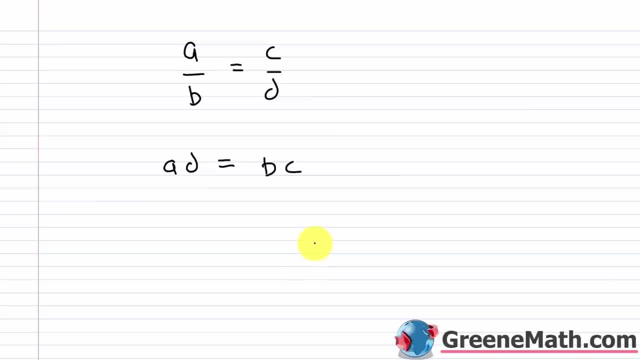 where did this cross-multiplication come from? Well, if I kind of look at the denominators here, I have b and I have d. So let's say I multiply both sides of the equation by the LCD, which is bd right, B times d. I multiply this side by bd, which is perfectly legal. 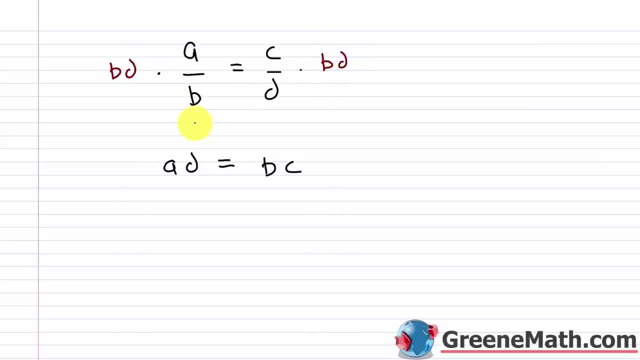 with an equation, as long as I do it to this side. We see here that this would cancel here, and we also see that this would cancel here. So what would I have left? I'd have d times a, which is the same as a. 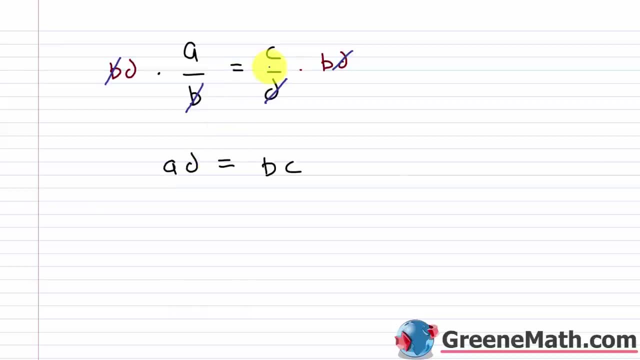 I just switched the order And this is equal to C times B or BC, right? So if I multiply both sides of the equation by the LCD, I end up with this right here. This is kind of just a shortcut, right? I'm multiplying this by this, and I'm multiplying this by this because the other part 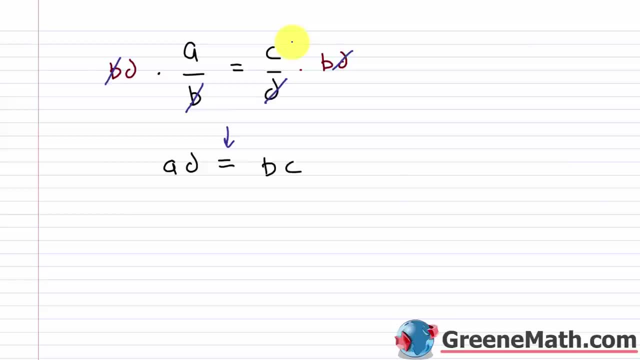 is going to cancel out. So I end up with AD equals BC. So we're going to be using this logic to solve a proportion equation. So here we have: 4 over 7 equals 2 over x. Now, in order to solve for the 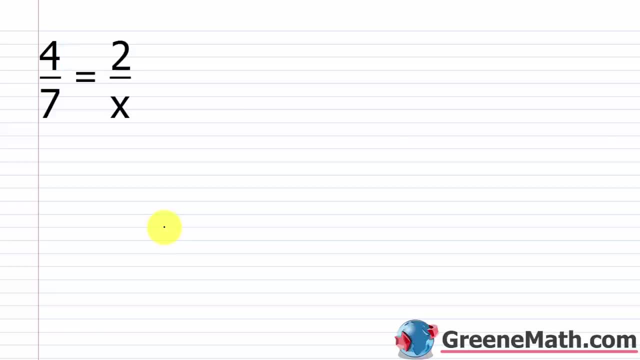 unknown in a proportion equation. we just remember that if it's true that 4: 7s equals 2 over x, that 7 times 2,, which is 14, 7 times 2, has to be equal to x times 4 or 4x. 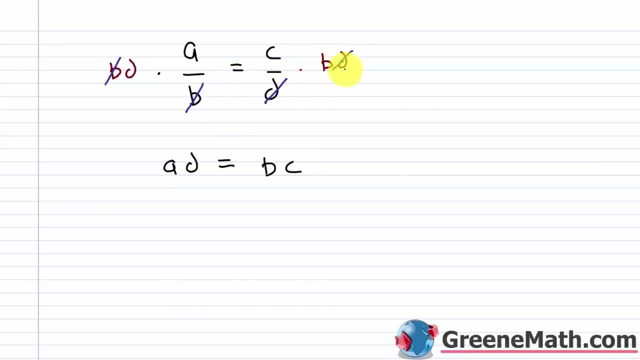 And this is equal to C times B, or BC. So, if I multiply both sides of the equation by the LCD, I end up with this right here. This is kind of just a shortcut. I'm multiplying this by this, and I'm multiplying this by this. 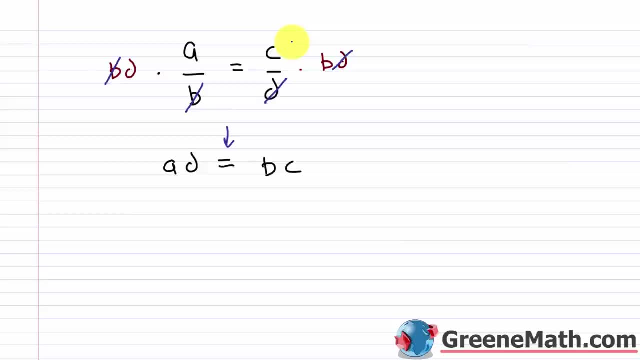 This part is going to cancel out. So, I end up with AD equals BC. So, we're going to be using this logic 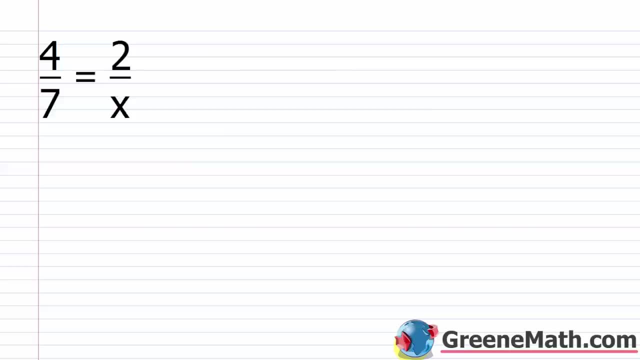 to solve a proportion equation. So, here we have 4 over 7 equals 2 over X. Now, in order to solve for the unknown in a proportion equation, 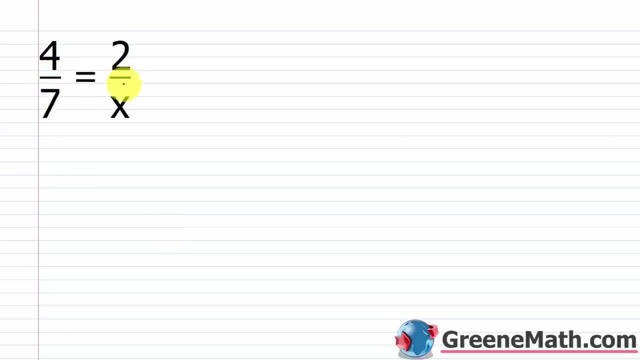 we just remember that if it's true that 4 sevenths equals 2 over X, that 7 times 2, which is 14, has to be equal to 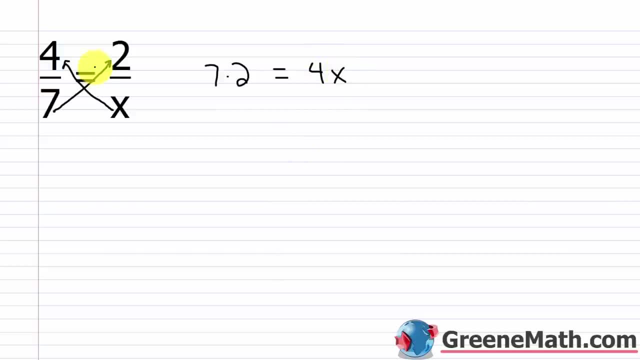 6 times 4, or 4X. Otherwise, we can't put an equal sign here. So, knowing that, I just cross multiply and set up an equation like I did here. This just becomes 14 is equal to 4X. And we simply solve for X. We divide both sides of the equation by 4. 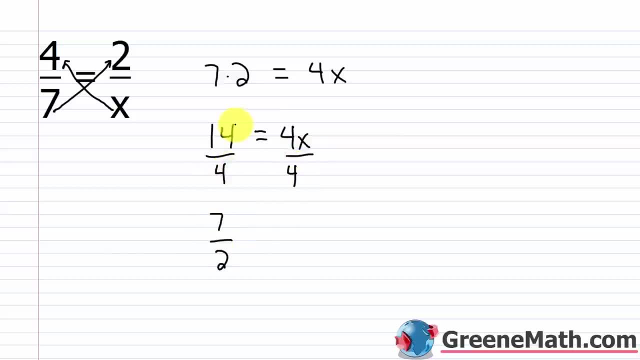 And we end up with 7 halves. If I divide 14 by 2, I get 7. If I divide 4 by 2, I get 2. 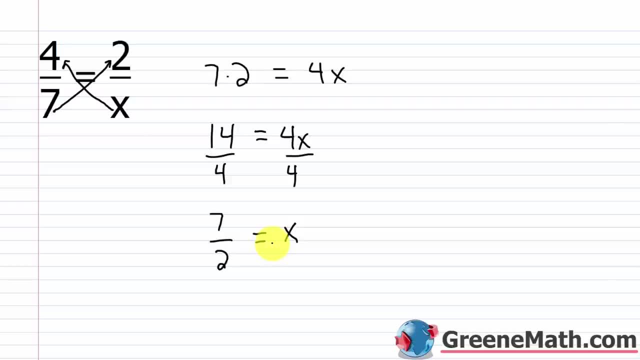 So, 7 halves equals X. Or, in decimal form, you could write but typically, if I'm working with 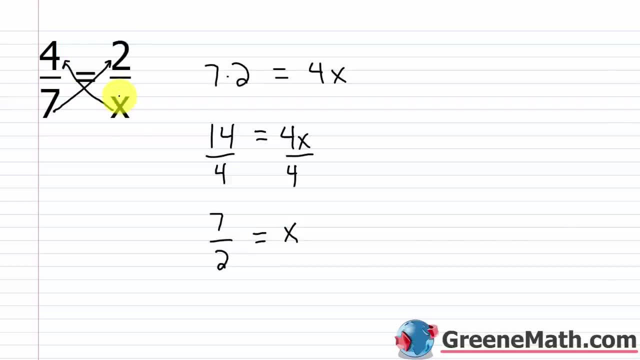 fractions or ratios or however you want to think about that, if I'm working with that, I want to stay with that. 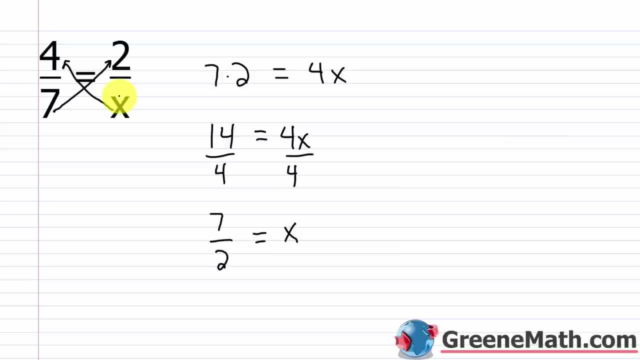 I don't want to switch to decimals. So, I get X equals 7 halves, or I have 7 halves equals X. 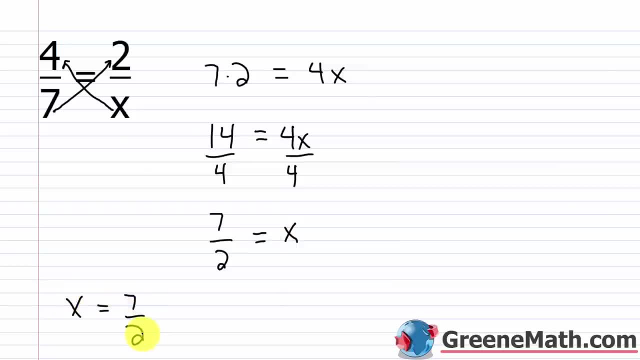 It doesn't really matter how you say that. And to check it, 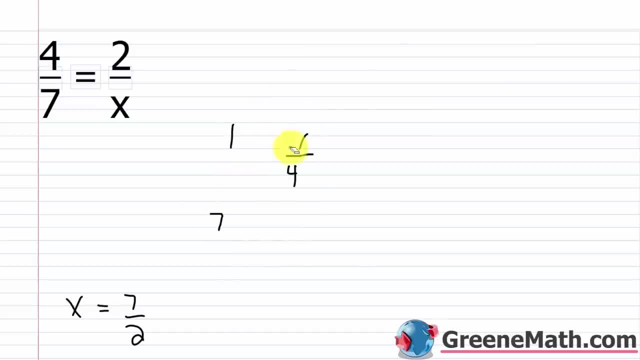 you just plug it in. I just plug in for X. So, what would I have? I'd have 4 sevenths is equal to 2, or I could write 2 as 2 over 1, divided by this X, which is 7 halves. 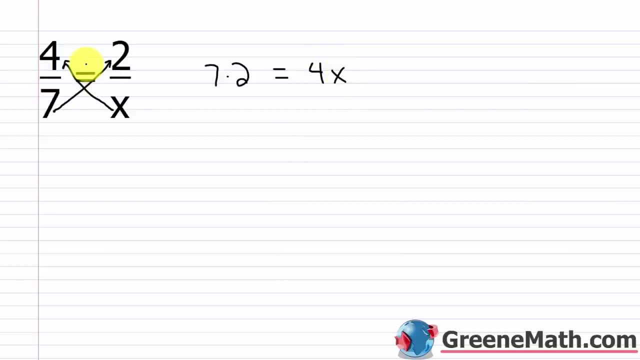 Otherwise we can't put an equal sign here. So, knowing that I just cross, multiply and set up an equation like I did here, This just becomes: 14 is equal to 4x, And we simply solve for x, We divide both sides of the equation by 4. And we end up with 7 halves. 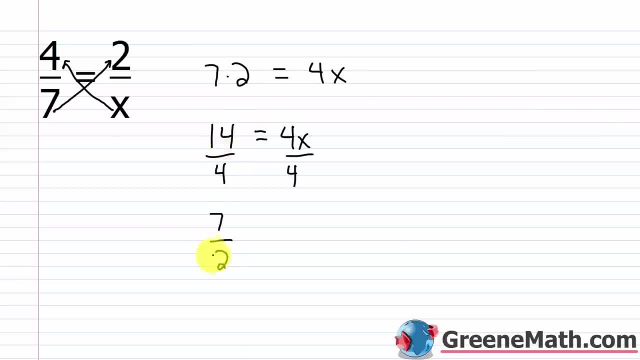 right. If I divide 14 by 2, I get 7.. If I divide 4 by 2,, I get 2.. So 7 halves equals x, Or in decimal form you could write 3.5.. But typically, if I'm working with fractions or 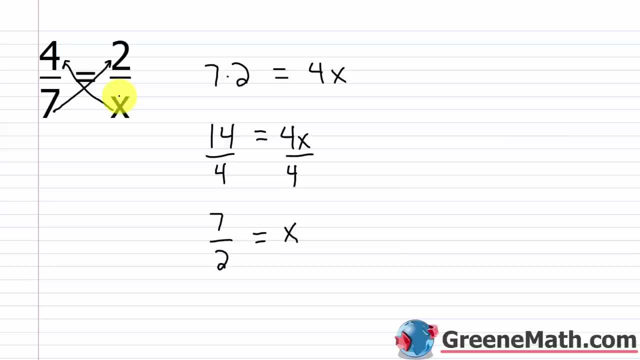 ratios or however you want to think about that. if I'm working with that, I want to stay with that. I don't want to switch to decimals. So I get x equals 7 halves, or I have 7 halves equals x. It. 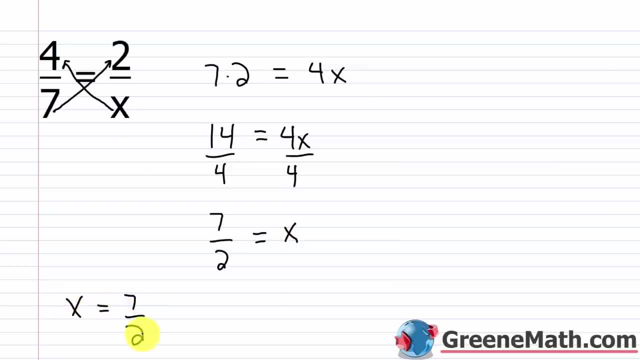 doesn't really matter how you say that, And to check it you just plug it in. I just plug in for x. So what would I have? I'd have 4. 7s is equal to 2, or I could write 2 as 2 over 1, divided by. 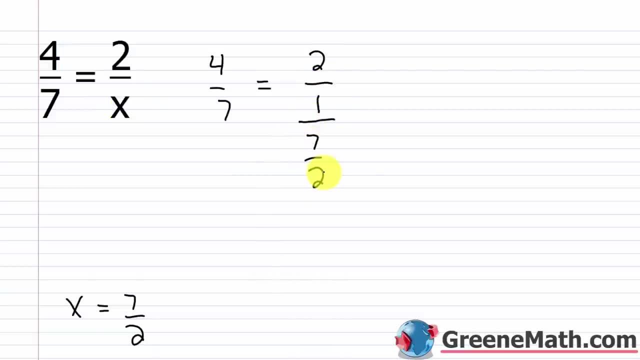 this x, which is 7 halves. And then it makes it obvious that I'm going to end up what I'm going to: take 2 over 1, and I'm going to multiply by the reciprocal of 7 halves, which is 2 over 7.. 2 times. 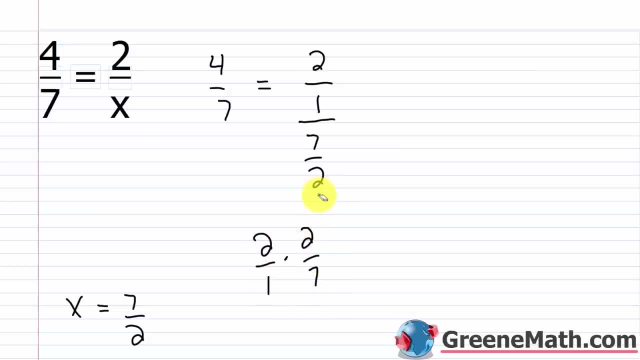 2 is 4 over 1 times 7, which is 7.. So this becomes 4 7ths as well. So we get that 4 7ths equals 4 7ths. Both sides are the same value, And so we know our solution: x equals 7 halves is correct. 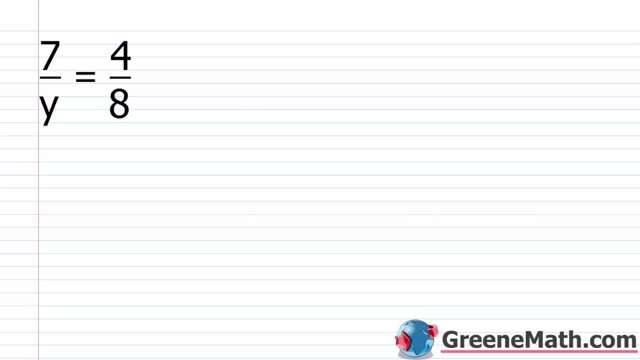 All right, let's take a look at another one. We have: 7 over y equals 4 8ths, or 4 over 8.. So again I'm going to cross, multiply and set up an equation: y times 4, which is just 4y, has to be equal to 8 times 7.. 8 times 7 is 56,. 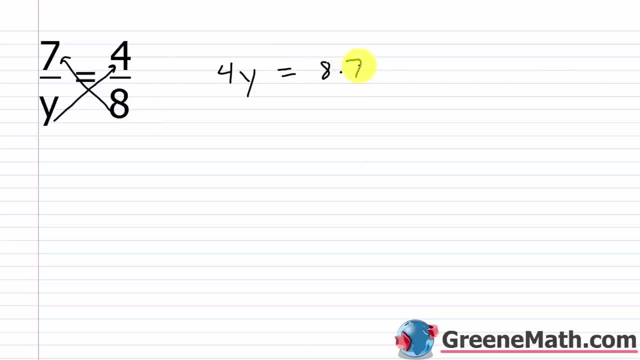 or I can write 8 times 7 and do it in two steps. So that's the first thing: Just cross, multiply, set up an equation. So then we have: 4y is equal to 56, right, 8 times 7 is 56. And then we just 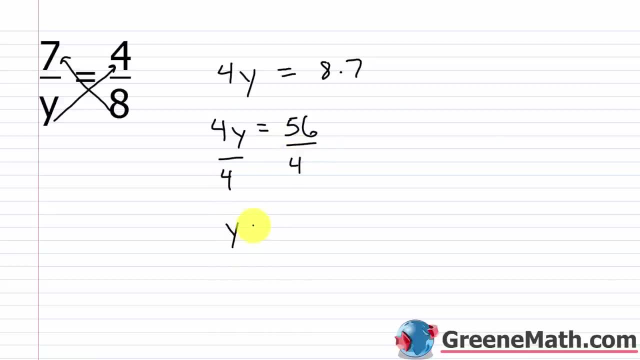 divide both sides of the equation by 4, the coefficient of y 56 divided by 4 is 14.. So we get 14 here. So y is equal to 8 times 7.. And then we just divide both sides of the equation by 4,. 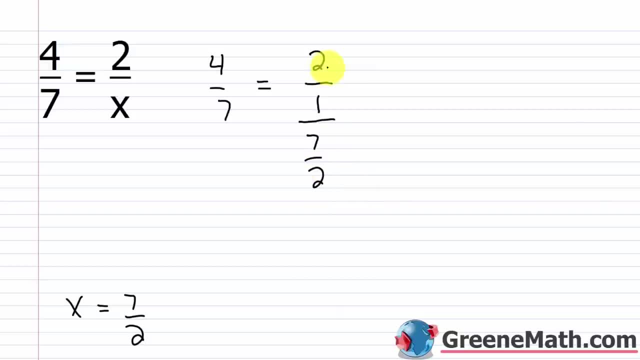 And then it makes it obvious that I'm going to end up what? I'm going to take 2 over 1, and I'm going to multiply by the reciprocal of 7 halves, which is 2 over 7. 2 times 2 is 4, over 1 times 7, which is 7. So, this becomes 4 sevenths as well. So, we get that 4 sevenths equals 4 sevenths. 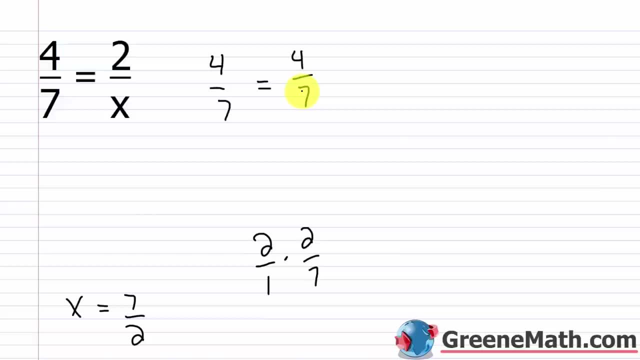 Both sides are the same value, and so we know our solution, X equals 7 halves, is correct. We have 7 over Y equals 4 eighths, or 4 over 8. 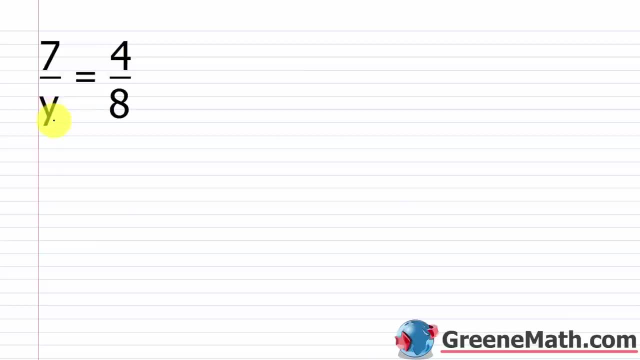 So, again, I'm going to cross multiply and set up an equation. Y times 4, which is just 4Y, has to be equal to 8 times 7. 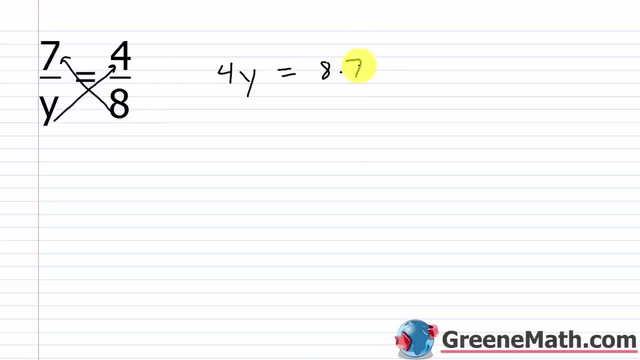 8 times 7 is 56, so I can write 8 times 7 and do it in 2 steps. 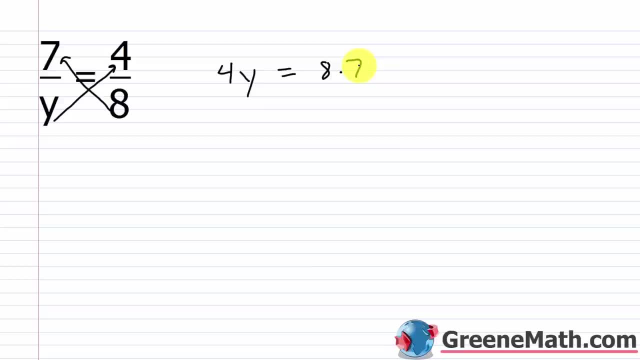 So, that's the first thing. Just cross multiply, set up an equation. 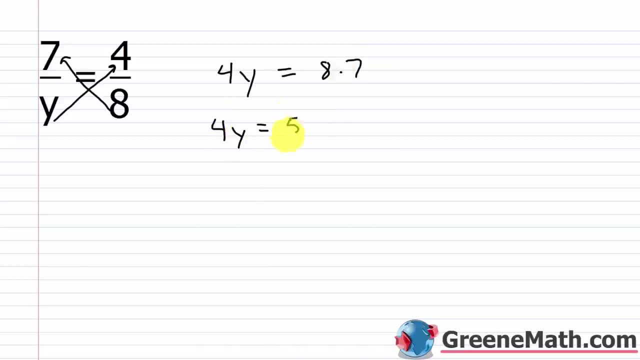 So, then we have 4Y is equal to 56, right? 8 times 7 is 56. And then we just divide both sides of the equation by 4, the coefficient of Y. 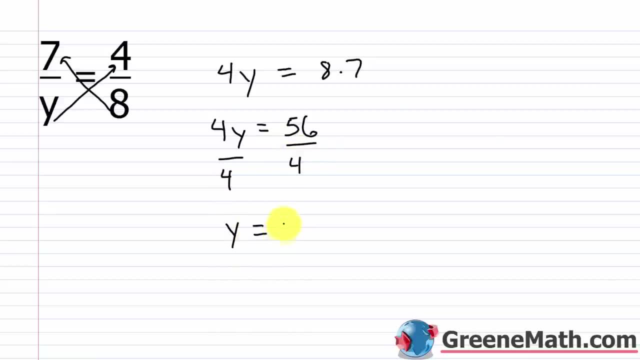 56 divided by 4 is 14. So, we get 14 here. So, Y equals 14. 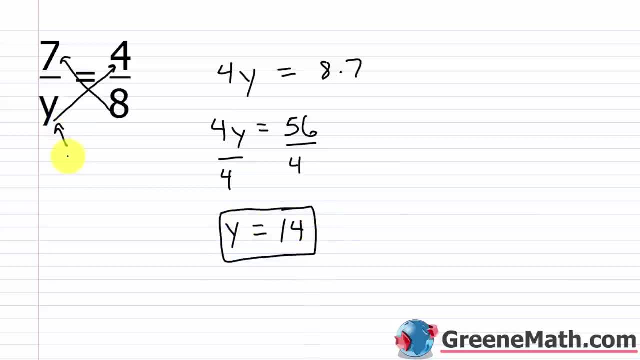 Alright. So, if I plug in a 14 for Y, you can mentally see that that's going to work out, right? Because 4 is half of 8, and 7 is half of 14. So, if I reduce each, if I divide 4 by 4, I get 1. If I divide 8 by 4, I get 2. 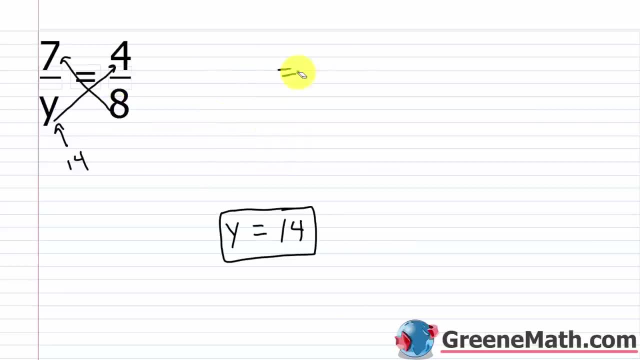 So, if I think about this, just as taking the fractions and simplifying them, 4 eighths is 1 half. 7 fourteenths is also 1 half, right? If I divide 7 by 7, I get 1. If I divide 14 by 7, I get 2. So, 1 half equals 1 half is what you'd end up with. And so, Y equals 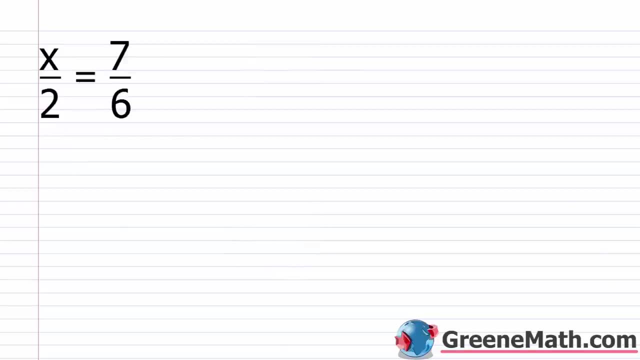 14 is the correct solution. Alright, now we want to take a look at X over 2 equals 7 sixths. 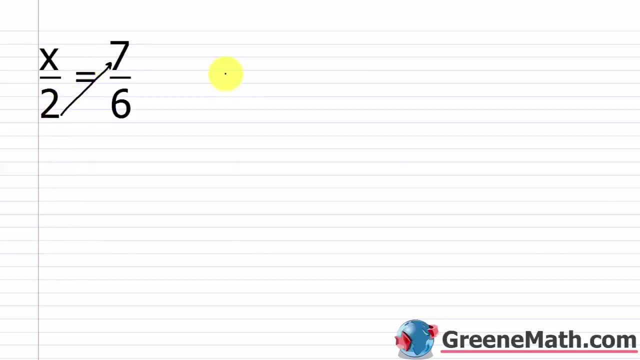 So, again, I'm just going to cross multiply and set up an equation. So, 2 times 7 is 14. 14. And that equals 6 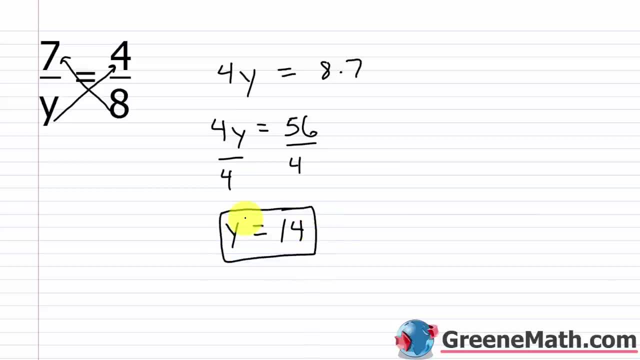 y equals 14.. All right, so if I plug in a 14 for y, you can mentally see that that's going to work out right, Because 4 is half of 8, and 7 is half of 14.. So if I reduce each, if I divide 4 by 4,, 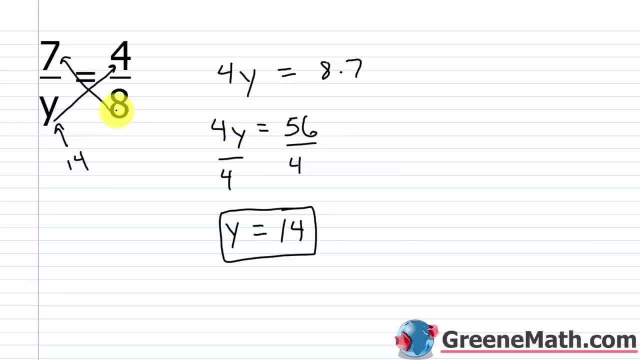 I get 1.. If I divide 8 by 4, I get 2, right. So if I think about this, just as taking the fractions and simplifying them, 4, 8ths is 1 half. 14ths is also 1 half, right. If I divide 7 by 7, I get 1.. If I divide 14 by 7, I get 2.. So 1 half. 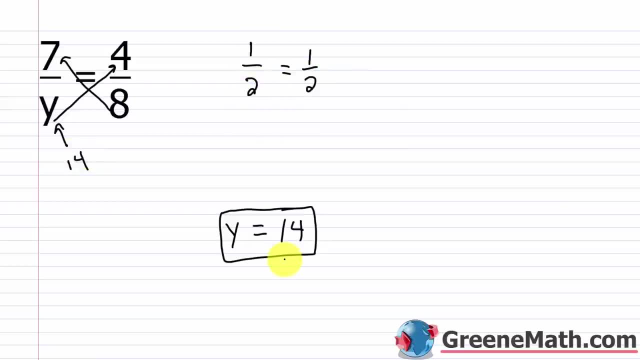 equals 1 half is what you'd end up with, And so y equals 14 is the correct solution. All right, now we want to take a look at x over 2 equals 7 6ths. So again, I'm just going to cross multiply. 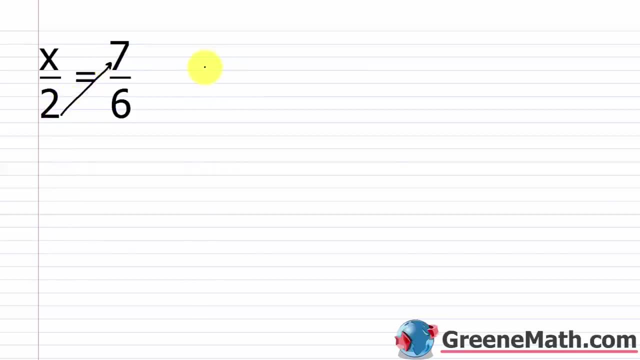 and set up an equation. So 2 times 7 is 14.. 14, and that equals 6 times x. that's 6x, All right. so once we've set up the equation, we're going to take a look at x over 2, and we're going to 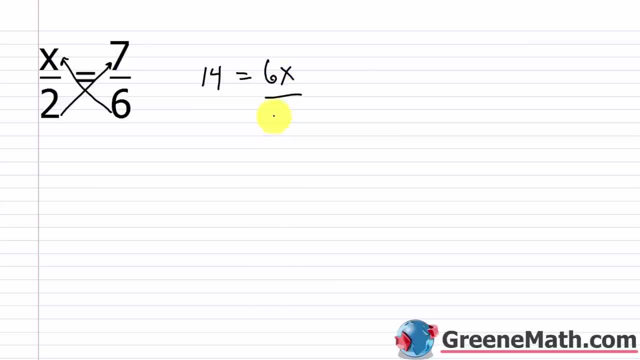 divide both sides of the equation by the coefficient of x, which is 6.. That will cancel with that and just leave me with x. What is 14 divided by 6?? Well, I can use a decimal, which, again, if I'm working with fractions or again, ratios, I just want to keep it in that form. 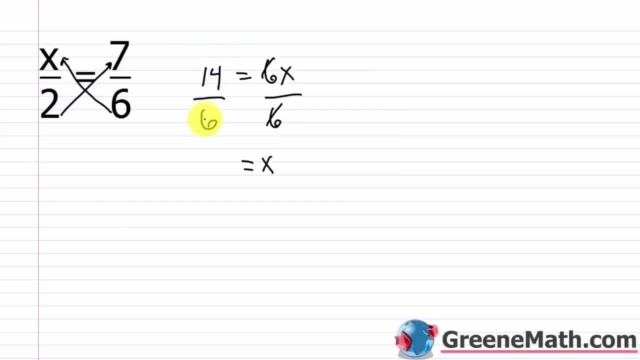 make it nice and simple. So I'm just going to simplify this, since I wouldn't get a whole number. Each is divisible by 2.. So this, divided by 2, is 7.. This, divided by 2, is 3.. So x is going. 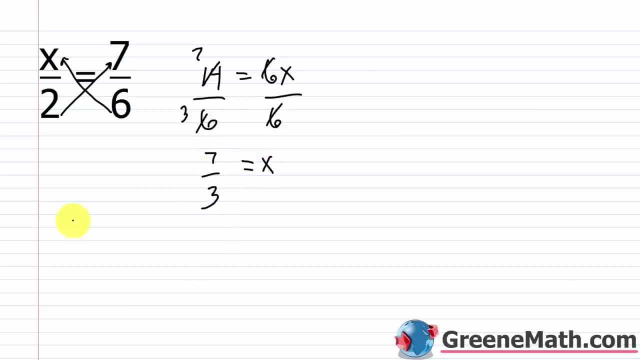 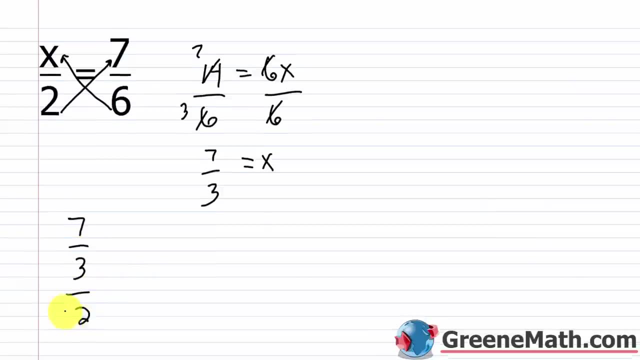 to equal 7 thirds, And again plug in for x there. So I'd have 7 thirds divided by 2.. So divided by 2.. And again, for the purpose of working with fractions, we'll say divided by 2 over 1.. And so I know. 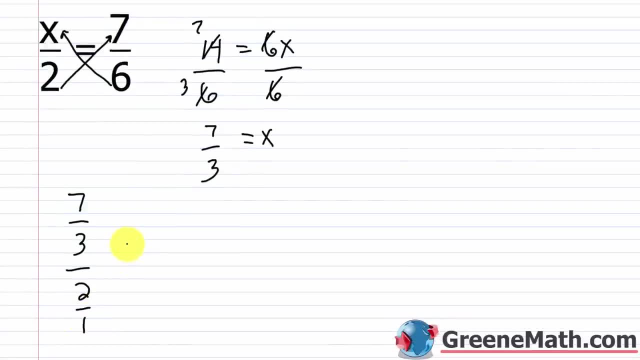 that that's basically 7 thirds times the reciprocal of 2 over 1.. So it's 7 thirds times 1. half 7 times 1 is 7, which is what I have up here. 3 times 2 is 6, which is what I have here. So I 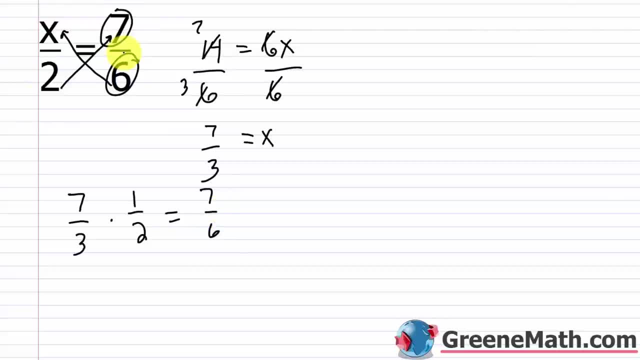 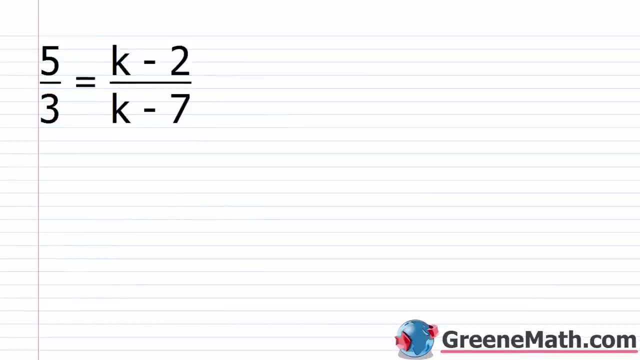 would get 7 6ths on the left as well as on the right. So again, x equals 7 thirds is my correct solution. All right, let's take a look at one that's a little bit harder, And by harder I just mean more tedious. So we have: 5 over. 3 is equal to k minus. 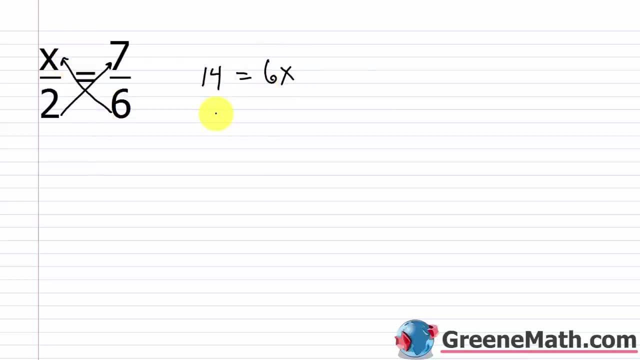 times X. That's 6X. Alright, so once we've set up the equation, we just divide both sides of the equation by the coefficient of X, which is 6. That will cancel with that. Just leave me with X. 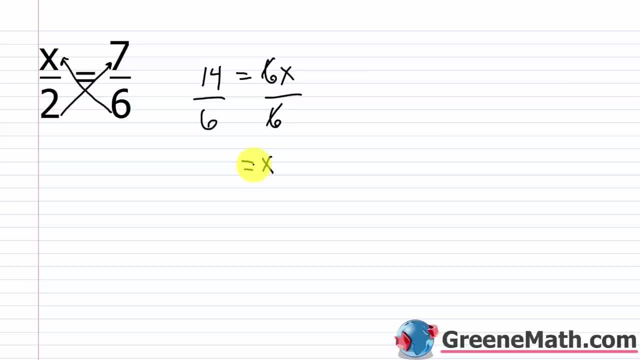 What is 14 divided by 6? Well, I can use a decimal, which, again, if I'm working with fractions or, again, ratios, I just want to keep it in that form. Make it nice and simple. So, I'm just going to simplify this since I wouldn't get a whole number. 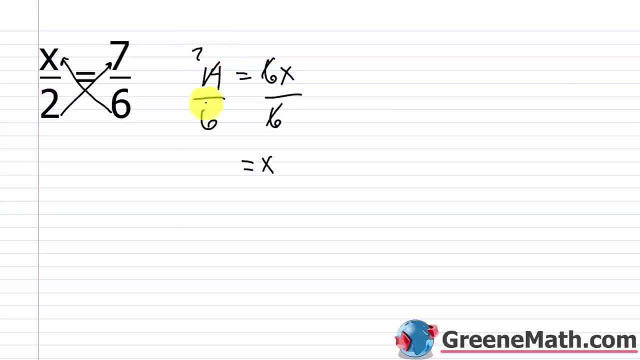 Each is divisible by 2. So, this divided by 2 is 7. 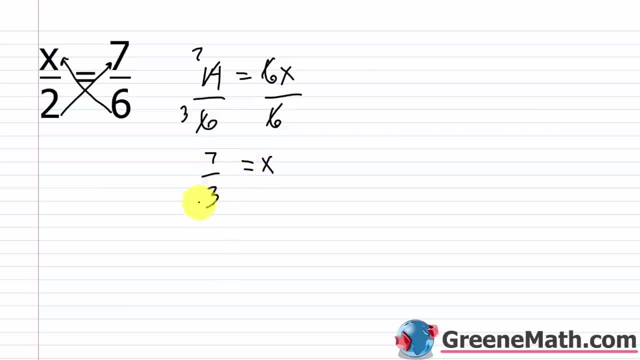 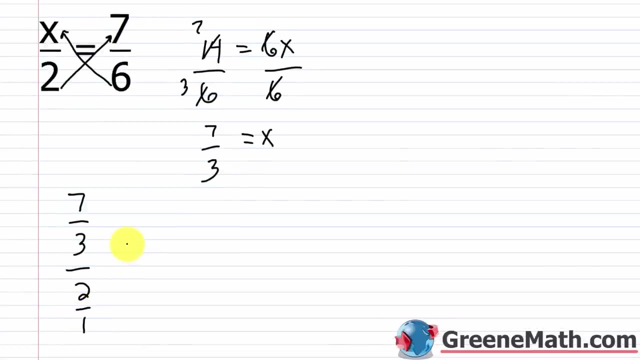 This divided by 2 is 3. So, X is going to equal 7 thirds. And, again, plug in for X there. So, I'd have 7 thirds divided by 2. So, divided by 2. And, again, for the purposes of working with fractions, we'll say divided by 2 over 1. And so, I know that that's basically 7 thirds times the reciprocal of 2 over 1. 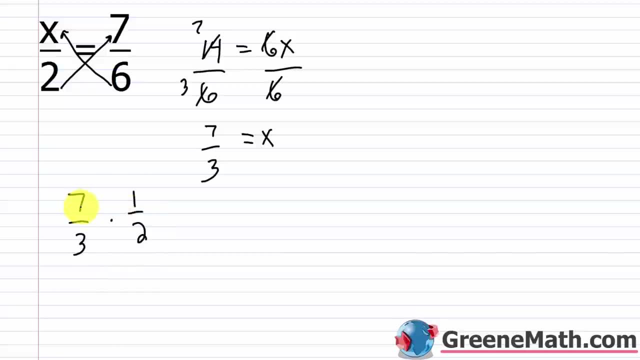 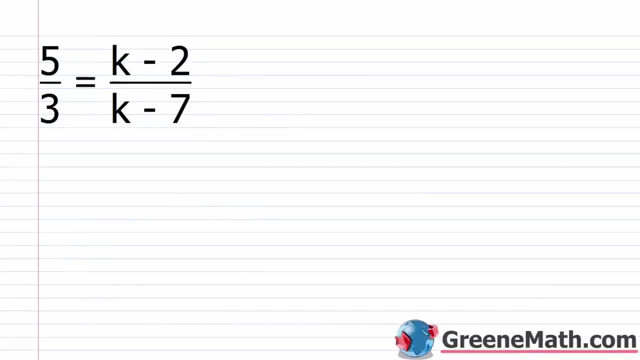 So, it's 7 thirds times 1 half. 7 times 1 is 7, which is what I have up here. 3 times 2 is 6, which is what I have here. So, I would get 7 sixths on the left as well as on the right. So, again, X equals 7 thirds is my correct solution. Alright, let's take a look at one that's a little bit harder. And, by harder, I just mean more tedious. 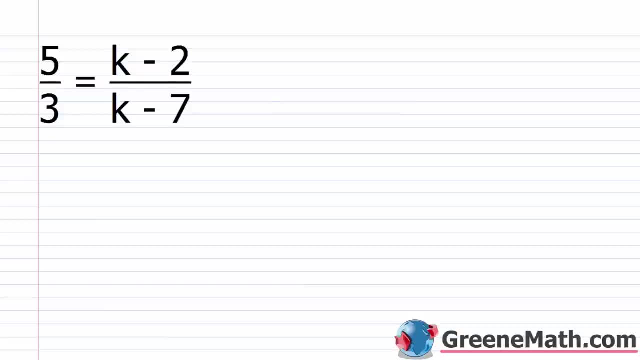 So, we have 5 over 3 is equal to k minus 2 over k minus 7. So, I'm doing the same thing. I'm going to take 3 and multiply it by this side. Now, very, very important here. I am multiplying 3 by this whole quantity. 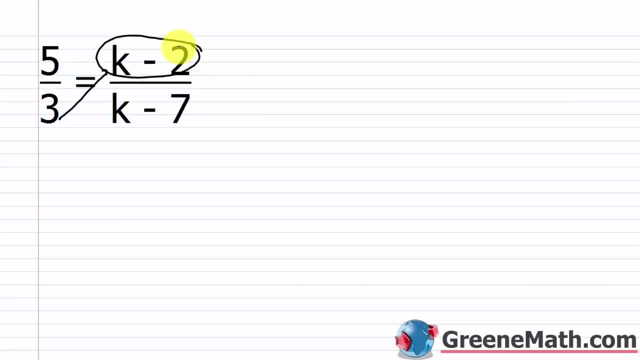 So, I need to use parentheses around that quantity. I need to say that 3 is going to be multiplied by 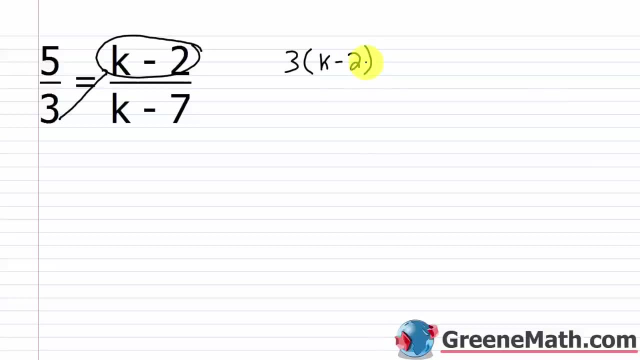 k minus 2. If I just put 3k minus 2 like that, I'm wrong. Because I didn't multiply 3 by 2. 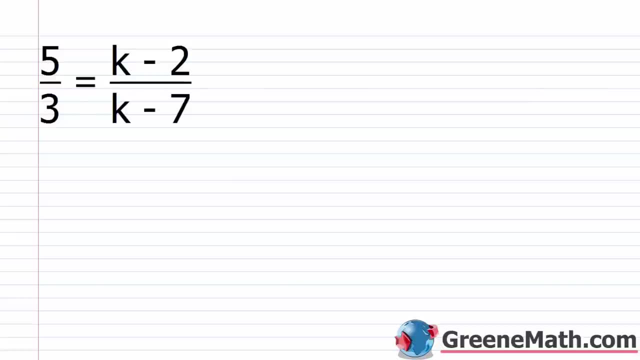 2 over k minus 7.. So I'm doing the same thing. I'm going to take 3 and multiply it by this side. Now, very, very important here I am multiplying 3 by this whole quantity, So I need to use. 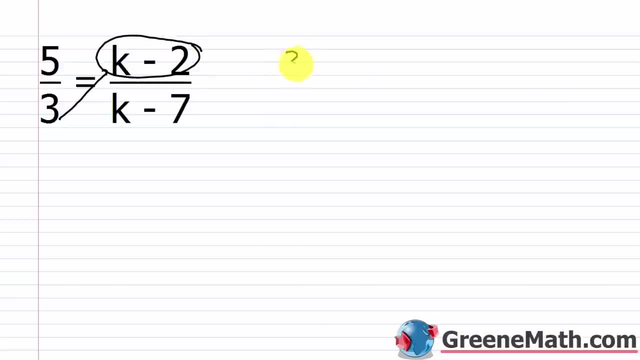 parentheses around that quantity. I need to say that 3, is going to be multiplied by k minus 2.. If I just put 3k minus 2 like that, I'm wrong, because I didn't multiply 3 by 2, right? So I need to make sure that 3 is multiplied by each term. 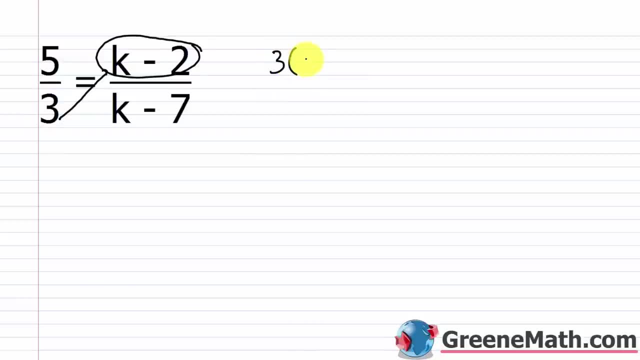 here And to do that again I use parentheses. So 3 times the quantity k minus 2 is equal to. I'm going to have this value multiplied by this, So 5 times the quantity k minus 7.. Again, you got to use parentheses. You're multiplying 5 by k and by negative 7.. So 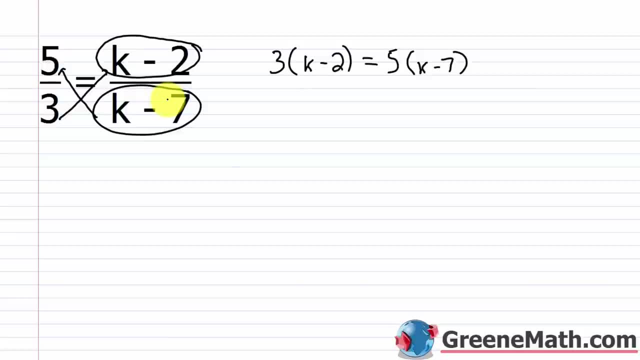 you use parentheses for that. Please don't make that mistake of not putting parentheses and not multiplying that number by each term: Very, very common, And it will cost you an answer on your test. All right, so now we simplify. So 3 times k is 3k, minus 3 times 2 is 6.. And this 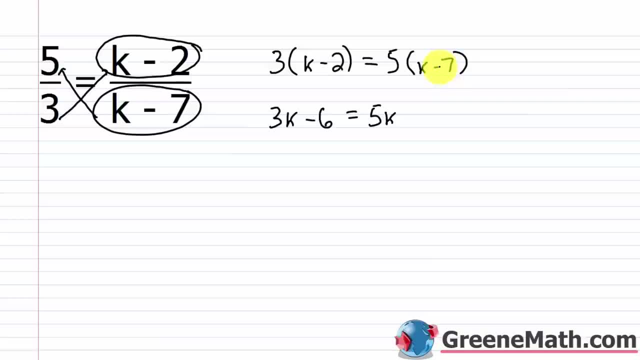 equals: 5 times k is 5k, Then 5 times negative 7 is negative 35. So now this is pretty easy to solve. I'm going to subtract 5k away from both sides. That way I just have a variable term on the left, nothing on the. 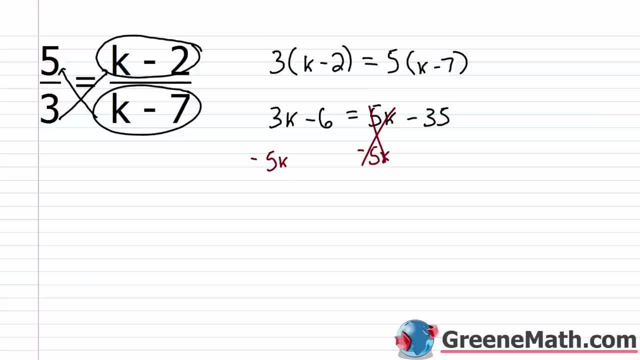 right. So this will go away And I'm going to end up with- I'm just going to kind of drag this over here- 3k minus 5k is negative 2k, And then minus 6 equals negative 35. I want to isolate this on. 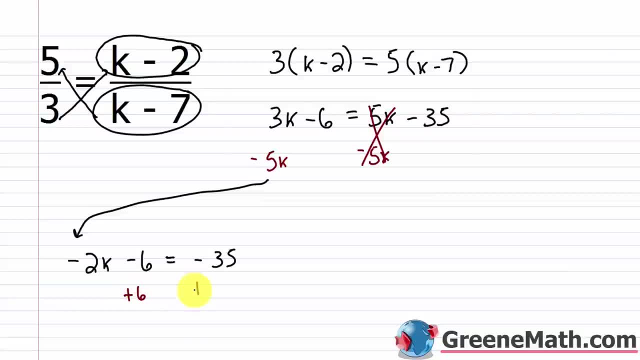 one side of the equation. So I'm going to add 6 to both sides. So I'm going to add 6 to both sides. So this is gone, And what I'm left with over here is negative 2k And, on the right, negative 35 plus. 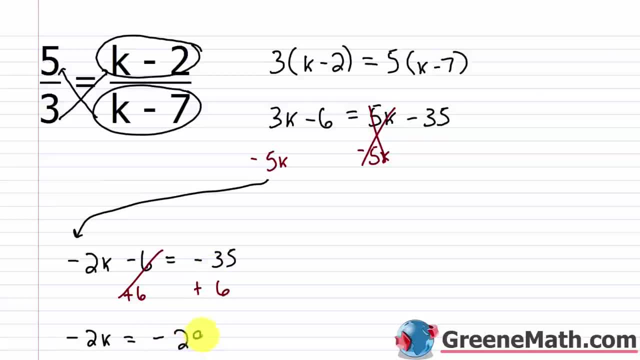 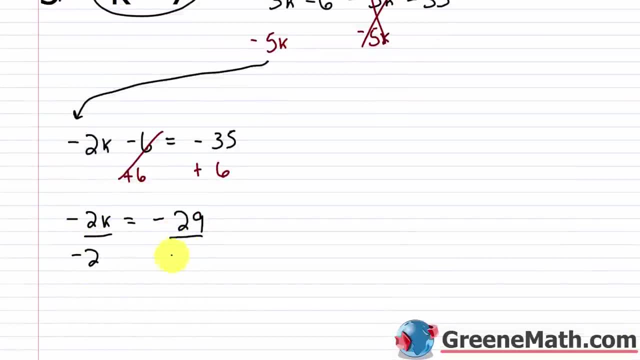 6 is going to be negative 29.. Okay, so continuing. I want k by itself. So I just divide both sides of the equation by negative 2, the coefficient of k. That cancels with that I have k over on the left. 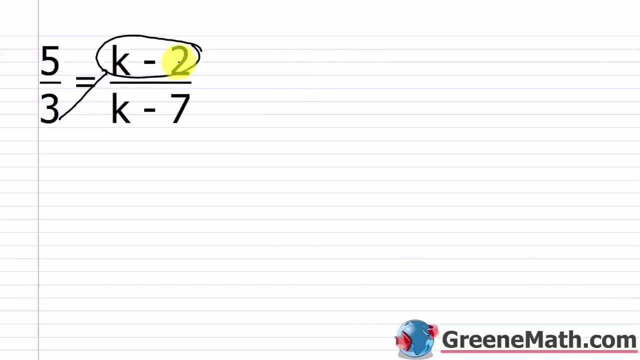 Right? So, I need to make sure that 3 is multiplied by each term here. And to do that, again, I use parentheses. So, 3 times the quantity k minus 2. Is equal to I'm going to have this value multiplied by this. So, 5 times the quantity k minus 7. 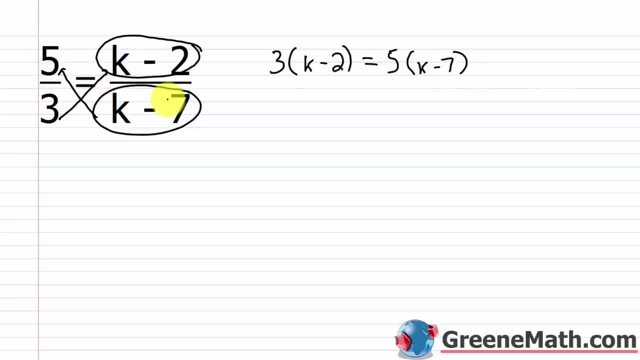 Again, you've got to use parentheses. You're multiplying 5 by k and by negative 7. So, you use parentheses for that. Please don't make that mistake of not putting parentheses and not multiplying that number by each term. Very, very common. And it will cost you an answer on your test. 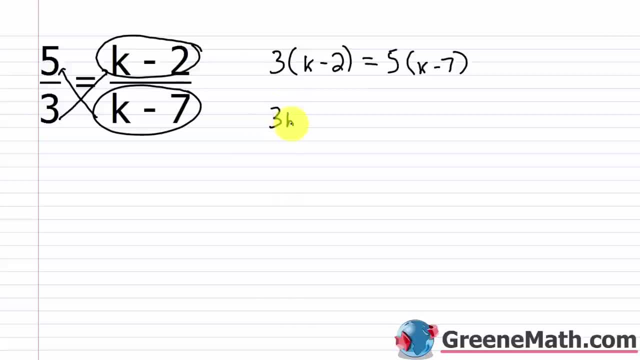 Alright. So, now we simplify. 3k is 3k. Minus 3 times 2 is 6. And this equals 5 times k is 5k. Then 5 times negative 7 is negative 35. So, now this is pretty easy to solve. I'm going to subtract 5k away from both sides. 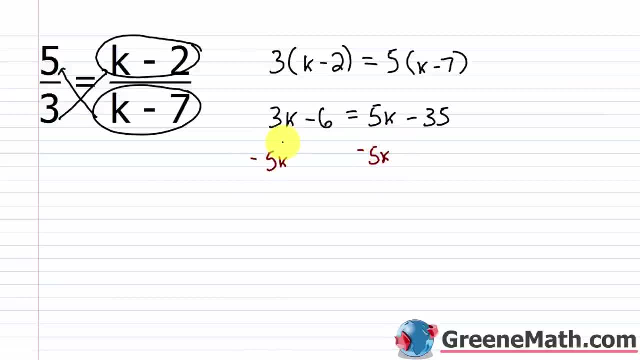 That way I just have a variable term on the left. Nothing on the right. 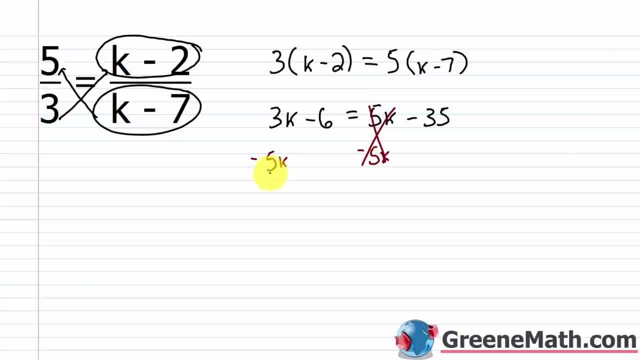 So, this will go away. And I'm going to end up with 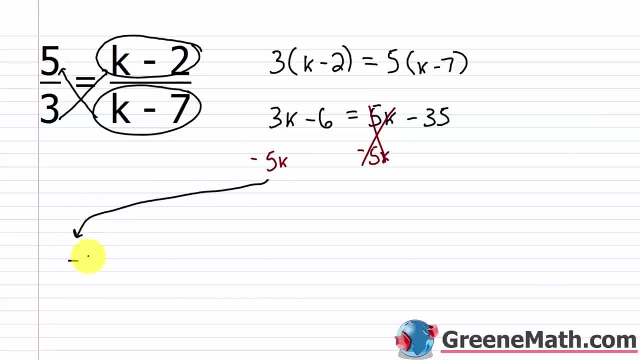 I'm just going to kind of drag this over here. 3k minus 5k is negative 2k. And then minus 6 equals negative 35. 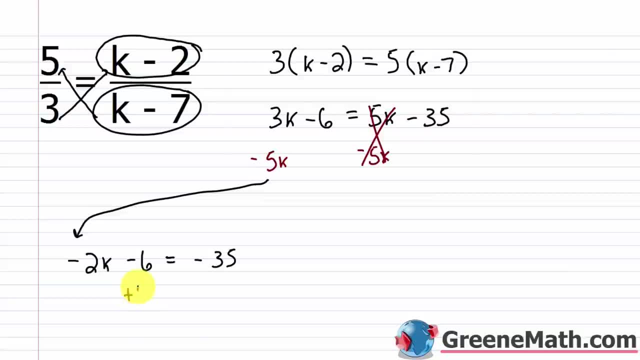 I want to isolate this on one side of the equation. So, I'm going to add 6 to both sides. So, this is gone. And what I'm left with over here is negative 2k. And on the right, negative 35 plus 6 is going to be negative 29. Okay. So, continuing. 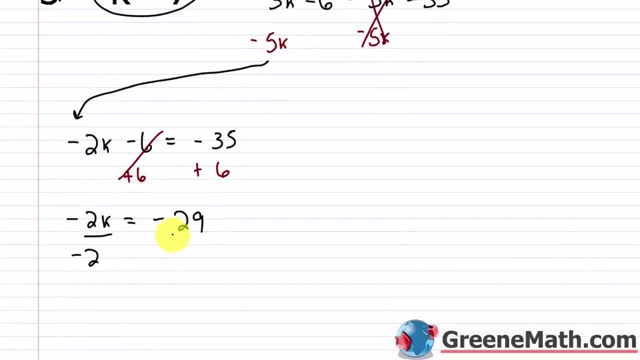 I want k by itself. So, I just divide both sides of the equation by negative 2. The coefficient of k. Cancels with that. I have k over on the left. On the right, I have negative 29 divided by negative 2. And 29 is a prime number. I would just leave it as 29 over 2. 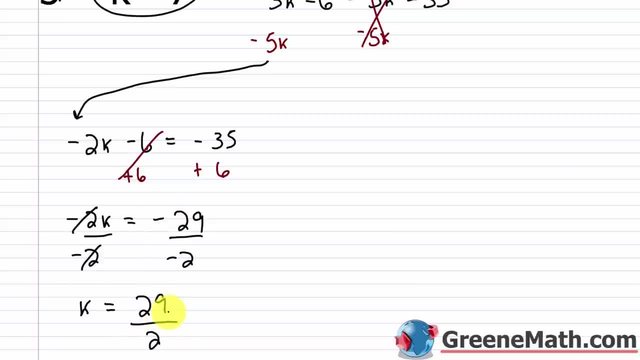 Right. Negative divided by negative is positive. So, you can remove the negative signs and list that it's positive. 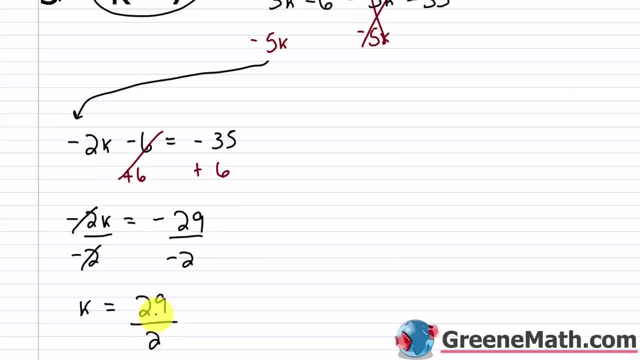 But you really can't simplify it any further. Now, checking this will be a little tedious. But we want to do it anyway. 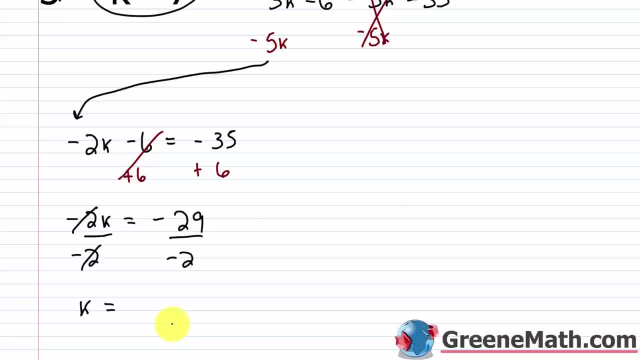 On the right I have negative 29 divided by negative 2. And 29 is a prime number. I would just leave it as 29 over 2.. Right Negative divided by negative is positive. So you can remove the negative signs and list that it's positive. but you really can't. 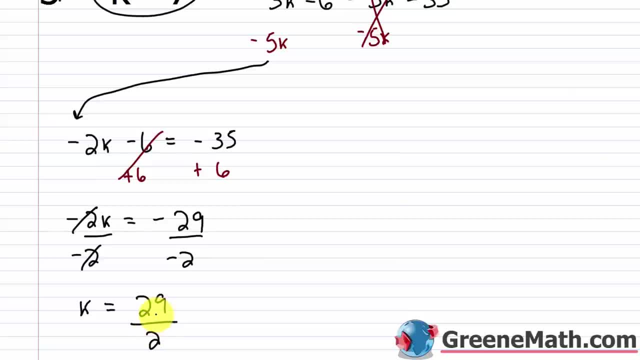 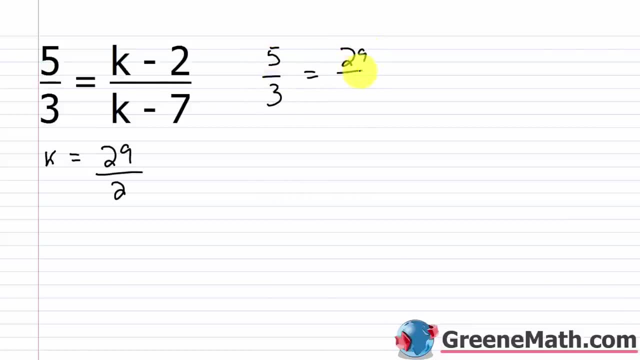 simplify it any further. Now checking this will be a little tedious, but we want to do it anyway. All right, so I would have 5 thirds equals. we have 29 halves minus 2.. And I'm going to go ahead and write 2 as 4 over 2.. So I have a common denominator And then this is over. 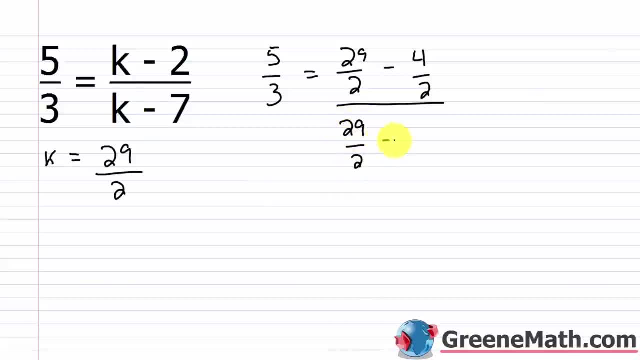 Again, for k, we have 29 over 2.. And then minus we have 7.. I'm going to go ahead and write that as 14 over 2. Again, so I have a common denominator. So this is basically what A complex fraction over here. 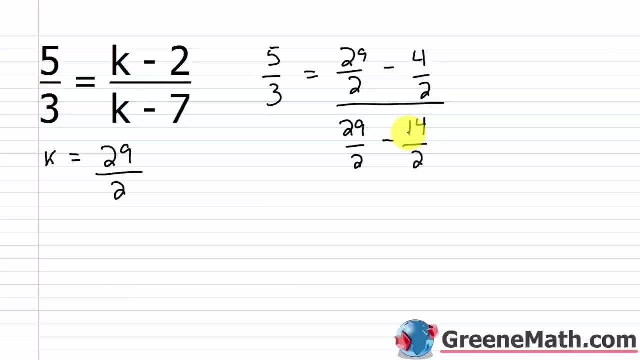 We already know how to simplify a complex fraction. Essentially, there's two different ways. We could multiply the numerator and the denominator of the complex fraction by the LCD, which would be 2.. Or we could just simplify the numerator and denominator separately. 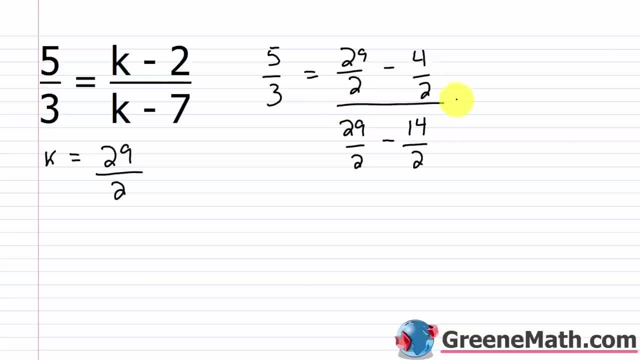 So I think it would be a little faster if we multiply the numerator and denominator here by 2.. So let's do that. So I'm going to multiply this by 2. And I'm going to multiply this by 2.. Now you might be thinking: oh, this is an equation, so I got to do this to the other side. 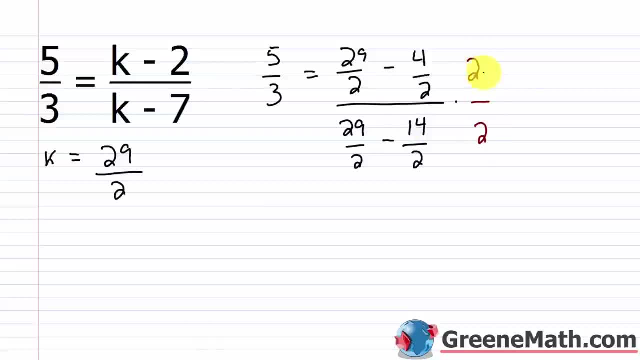 No, Remember, if I multiply a fraction by the same number, top and bottom, I don't change the value of that. I'm multiplying by 2 over 2, which is just basically I'm multiplying by 1.. If I multiply by, 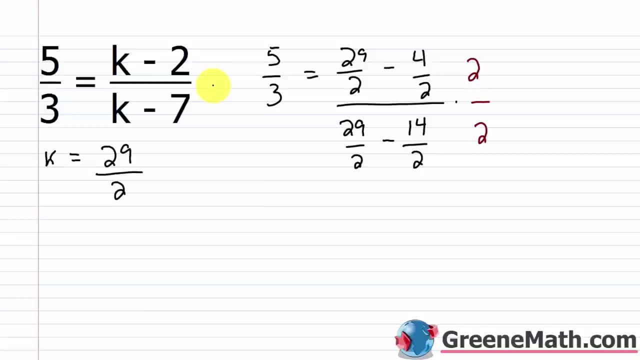 1 over here. I can multiply by 1 over here, but multiplying by 1 doesn't change the value of something, So I don't need to do that to both sides, I just need to do it to this side. This 2 is basically going to be distributed to this and it would cancel this 2 here. 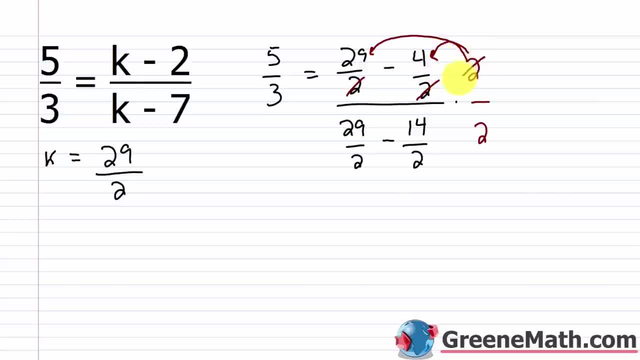 and then to this: and it would cancel this 2 here. So that's gone. Same thing over here. It would be distributed. This cancels, This cancels when it gets over here. So that's gone. So I can kind of erase the denominator. 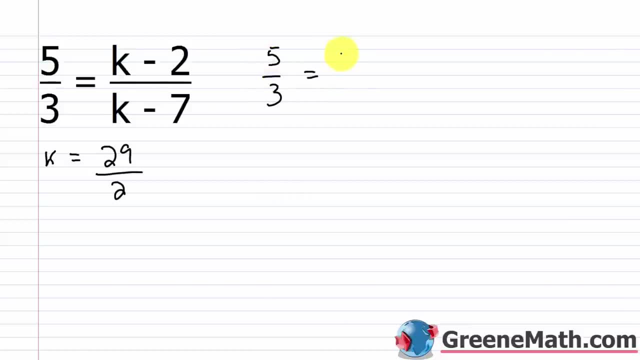 Alright. So, I would have 5 thirds equals 29 halves minus 2. And I'm going to go ahead and write 2 as 4 over 2. 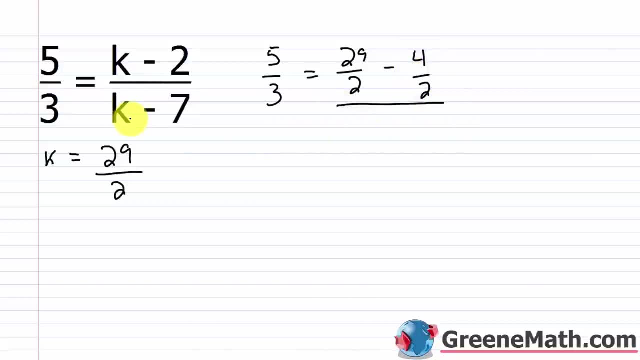 So, I have a common denominator. And then this is over. Again, for 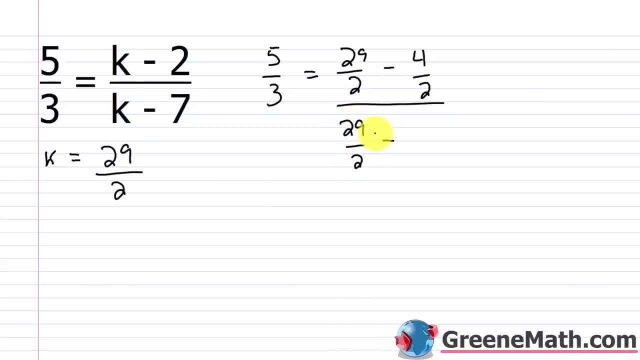 k, we have 29 over 2. And then minus, we have 7. I'm going to go ahead and write that as 14 over 2. Again, so I have a common denominator. So, this is basically what? A complex fraction over here. 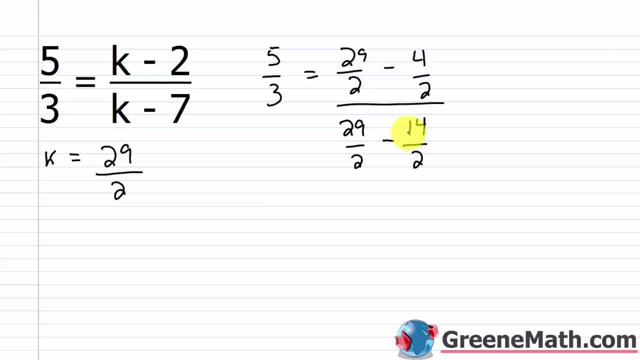 We already know how to simplify a complex fraction. 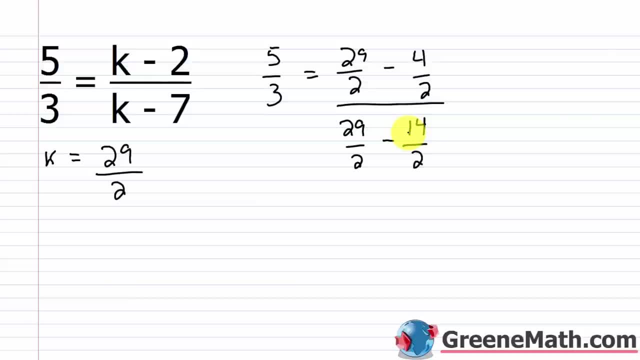 Essentially, there's two different ways. We could multiply the numerator and the denominator of the complex fraction by the LCD, which would be 2. Or, we could just simplify the numerator and denominator separately. So, I think it would be a little faster if we multiply the numerator and denominator here by 2. So, let's do that. 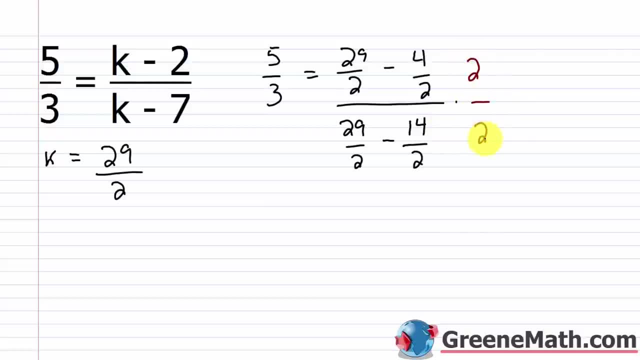 So, I'm going to multiply this by 2. And I'm going to multiply this by 2. Now, you might be thinking, oh, this is an equation, so I've got to do this to the other side. No. Remember, if I multiply a fraction by the same number, top and bottom, I don't change the value of that. I'm multiplying by 2 over 2, which is just basically I'm multiplying by 1. 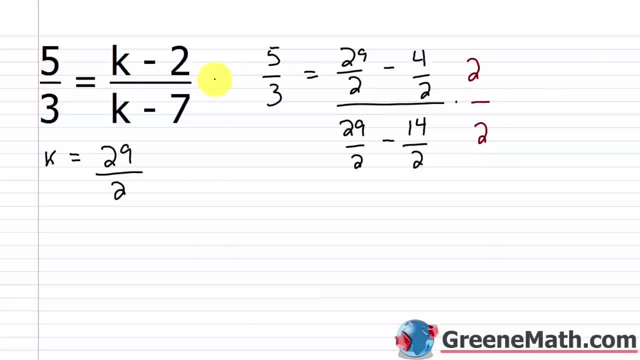 If I multiply by 1 over here, I can multiply by 1 over here, but multiplying by 1 doesn't change the value of something. So, I don't need to do that to both sides. I just need to do it to this side. This 2 is basically going to be distributed to this, and it would cancel this 2 here, and then to this, and it would cancel this 2 here. 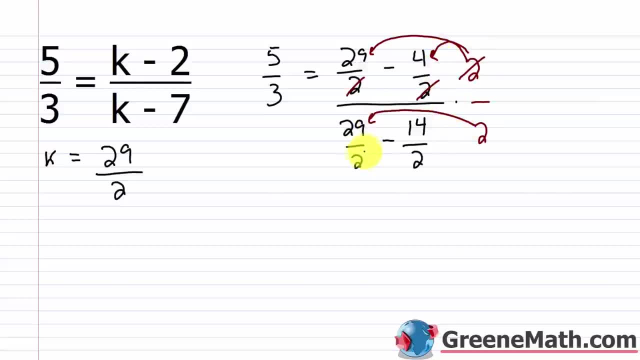 So, that's gone. Same thing over here. It would be distributed, this cancels, this cancels when it gets over here, so that's gone. 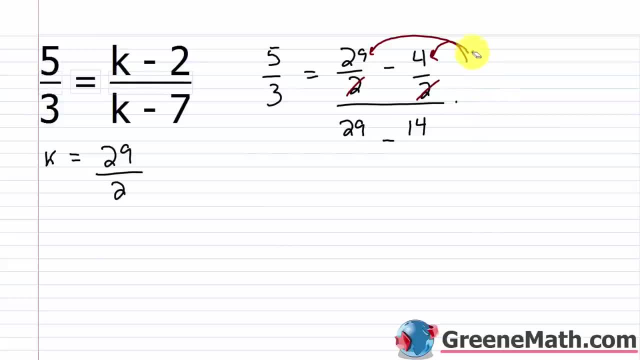 So, I can kind of erase the denominators here, because they would completely go away. So, this is gone, and essentially I'd have 29 minus 4, which is 25. 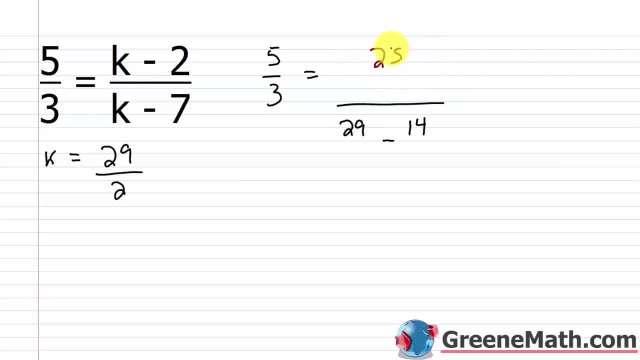 So, I could write this as 25, and then over 29 minus 14, which is 15. 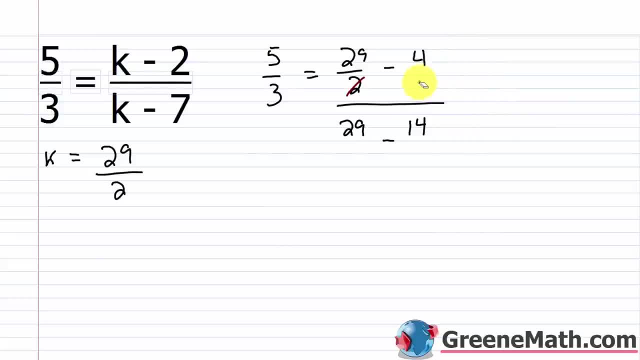 Here because they would completely go away. So this is gone And essentially I'd have 29 minus 4,, which is 25.. So I could write this as 25, and then over 29 minus 14,, which is 15.. 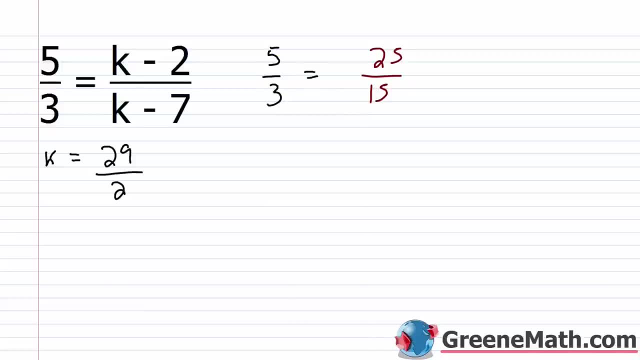 Now I can simplify this and make it look like this: 25 is divisible by 5.. 25 divided by 5 is 5.. 15 is divisible by 5.. 15 divided by 5 is 3.. So when I simplify 25 15ths, I end up with 5 3rds, So you get 5 3rds. 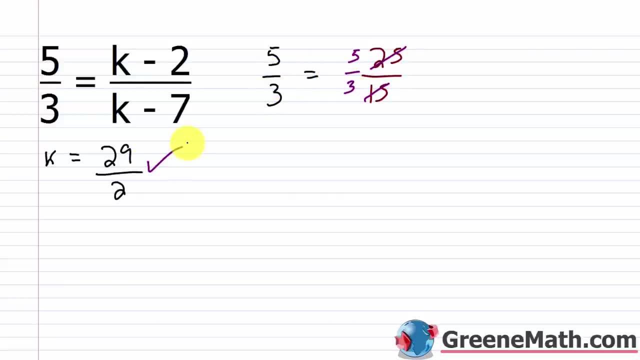 equals 5 3rds. So yeah, our solution- k equals 29 halves- is correct. All right, let's take a look at another one. We have 7 8ths equals v minus 7 over v plus 4.. So again set up your equation. 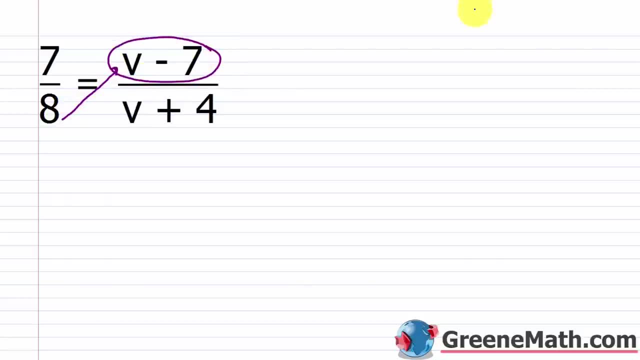 8 times this quantity v minus 7.. Again, have to use parentheses here, So I'm going to put: 8 times the quantity. 7 times the quantity v minus 7 is equal to this quantity v plus 4 times 7.. So again I got to use 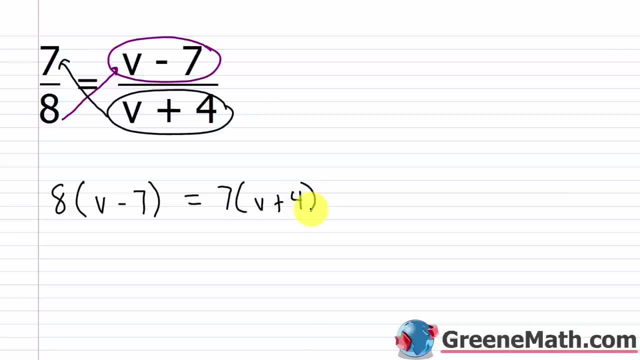 parentheses- 7 times the quantity v plus 4.. Again, 8 has to be multiplied by v and by negative 7.. All right, don't just do this. Don't just say okay, 8 times v minus 7.. That doesn't work. 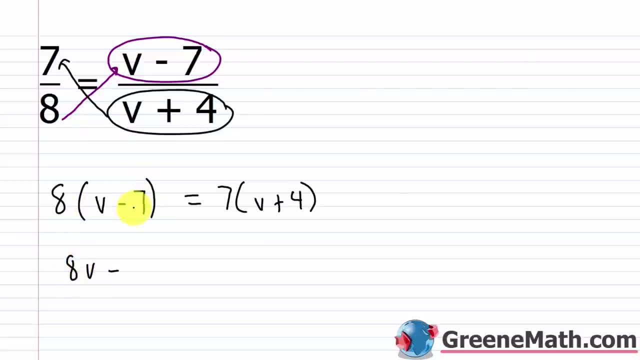 So 8 times v is 8v minus 8 times 7.. That's 56.. And this equals 7 times v, That's 7v Plus 7 times 4, that's 28.. All right, so I'm going to move my number to the right here. 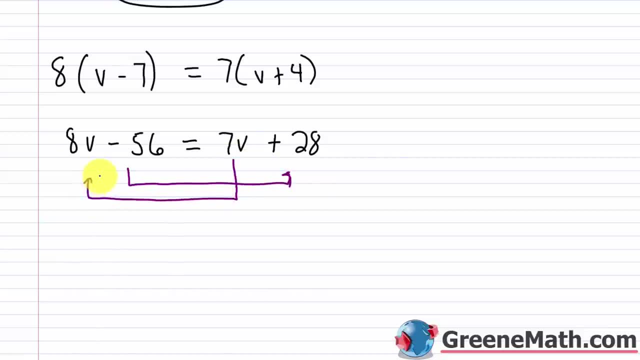 move my variable term to the left. Okay, and I'm going to do that in one step. So I'm going to add 56 to both sides of the equation. That way, there's no longer anything other than a variable term on the left. And I'm going to subtract 7v from both sides of the equation That way. 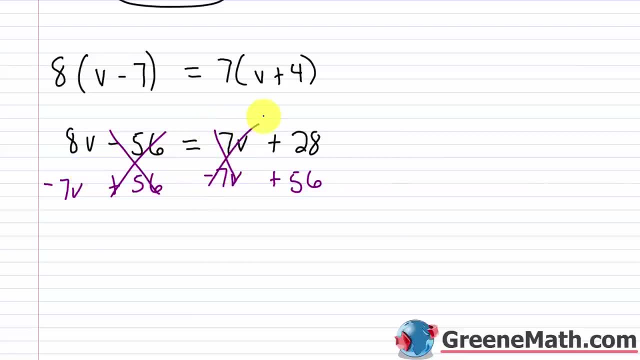 there's no longer a variable term on the left, So I'm going to subtract 7v from both sides of the equation. So on the left now I have 8v minus 7v, which is just v. On the right, I have 28 plus 56,. 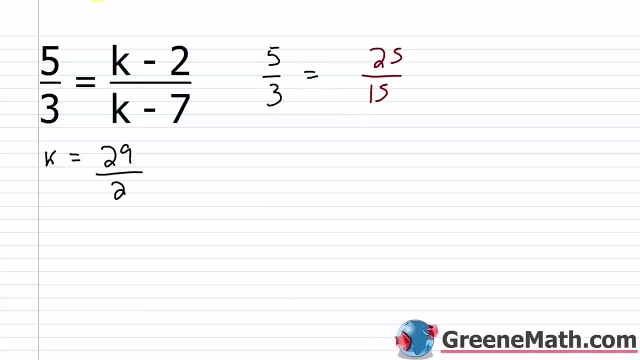 Now, I can simplify this and make it look like this. 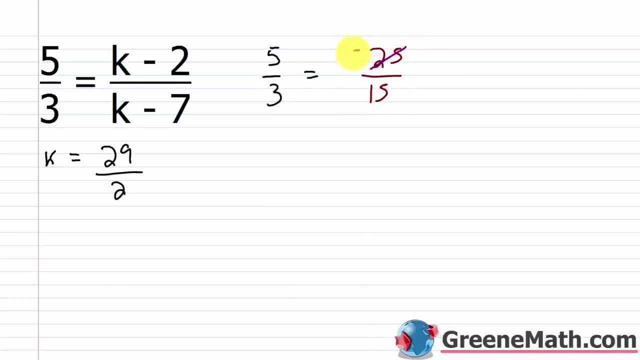 25 is divisible by 5. 25 divided by 5 is 5. 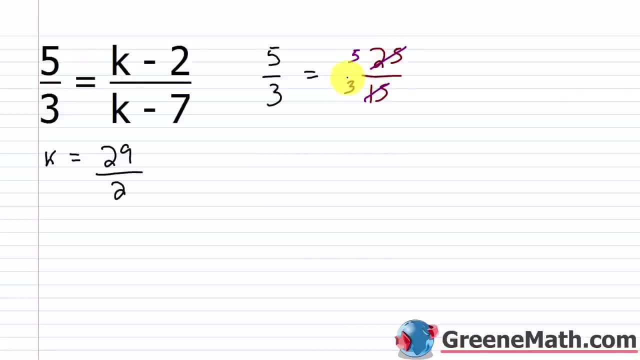 15 is divisible by 5. 15 divided by 5 is 3. So, when I simplify 25 15ths, I end up with 5 thirds. 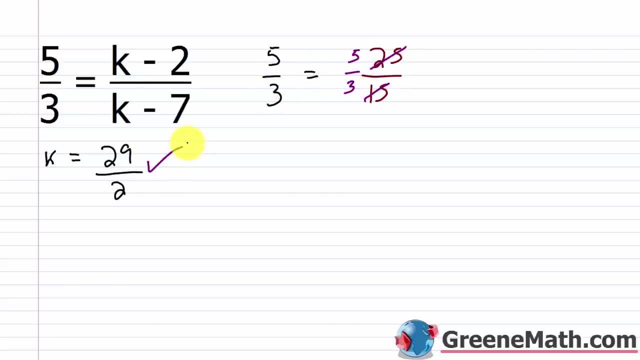 So, you get 5 thirds equals 5 thirds. So, yeah, our solution k equals 29 halves is correct. 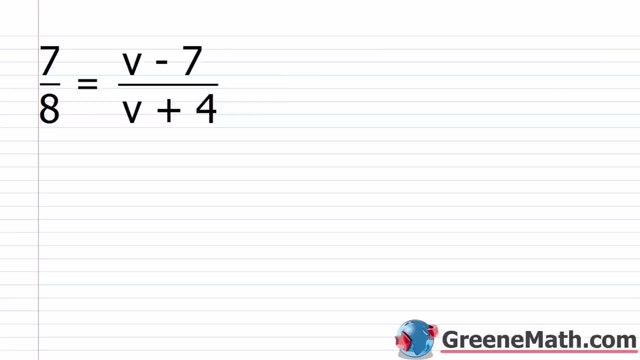 Alright, let's take a look at another one. We have 7 eighths equals 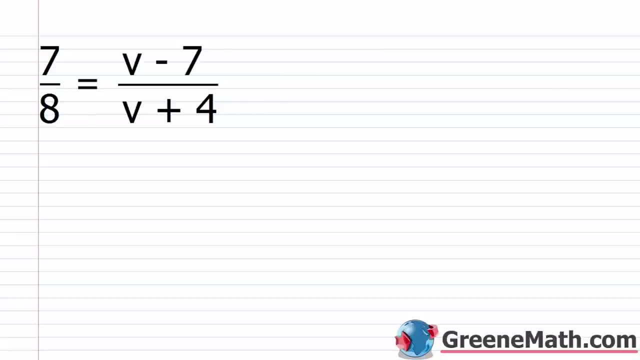 v minus 7 over v plus 4. 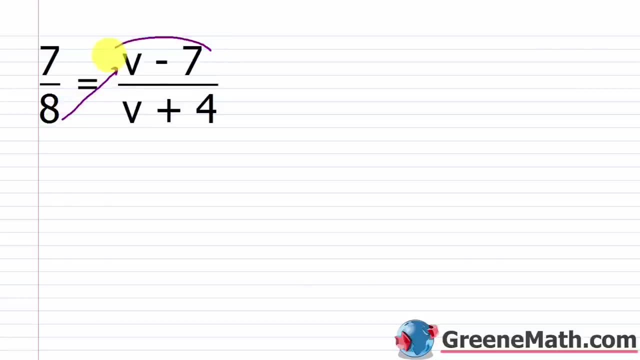 So, again, set up your equation. 8 times this quantity, v minus 7. Again, have to use parentheses here. So, I'm going to put 8 times the quantity v minus 7 is equal to this quantity, v plus 4, times 7. So, again, I've got to use parentheses. 7 times the quantity v plus 4. 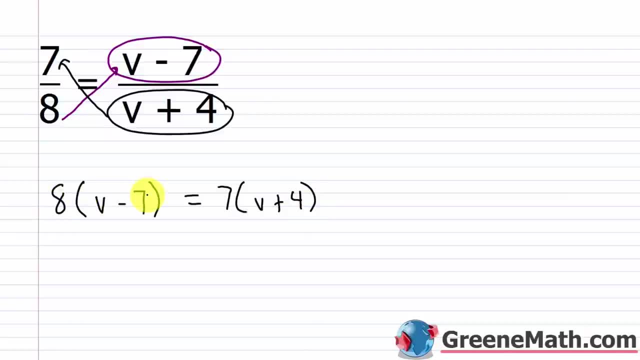 Again, 8 has to be multiplied by v and by negative 7. 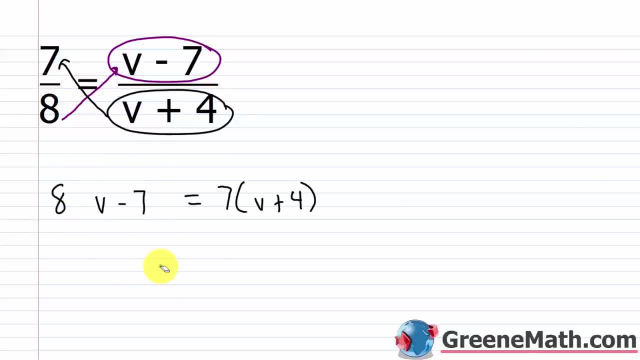 Alright, don't just do this. Don't just say, okay, 8 times v minus 7. 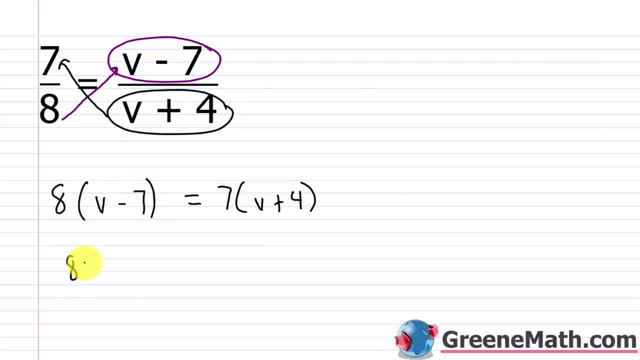 That doesn't work. So, 8 times v is 8v 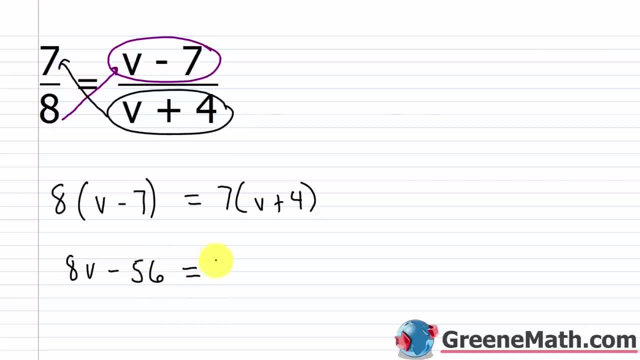 minus 8 times 7, that's 56. And this equals 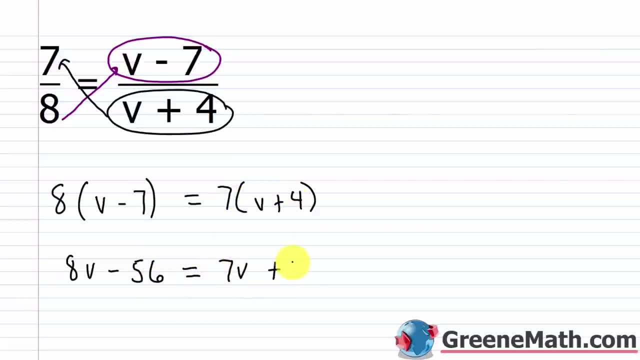 7 times v, that's 7v, plus 7 times 4, that's 28. Alright, so 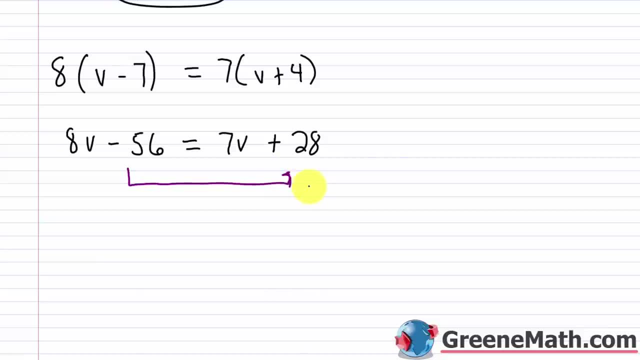 I'm going to move my number to the right here, move my variable term to the left. 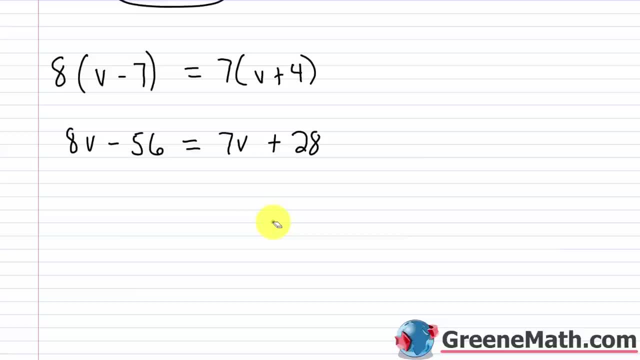 Okay? And I'm going to do that in one step. So, I'm going to add 56 to both sides of the equation. 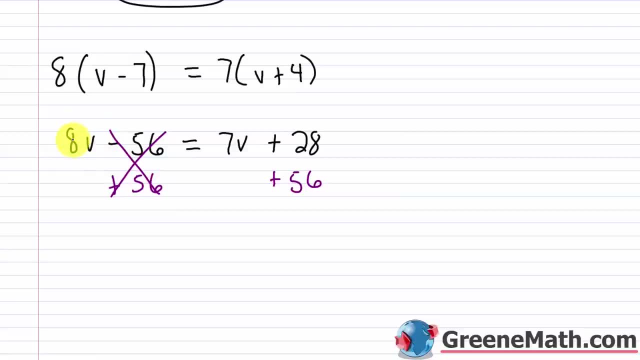 That way, there's no longer anything other than a variable term on the left. And I'm going to subtract 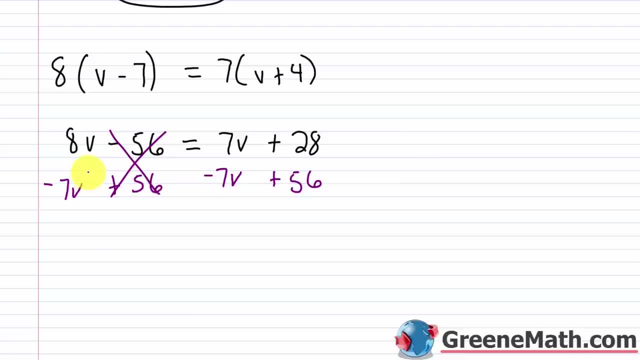 7v from both sides of the equation. That way, there's no longer a variable term on the right. So, on the left now, I have 8v minus 7v, which is just v. 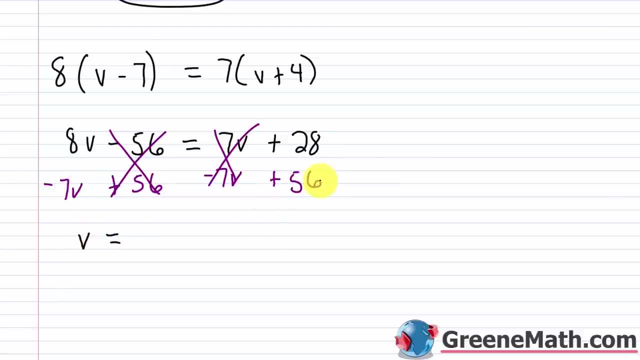 On the right, I have 28 plus 56, which is 84. Okay? So, v equals 84 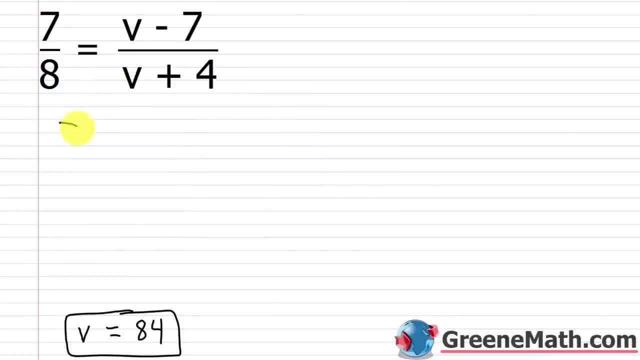 is our solution here. Alright, so we have 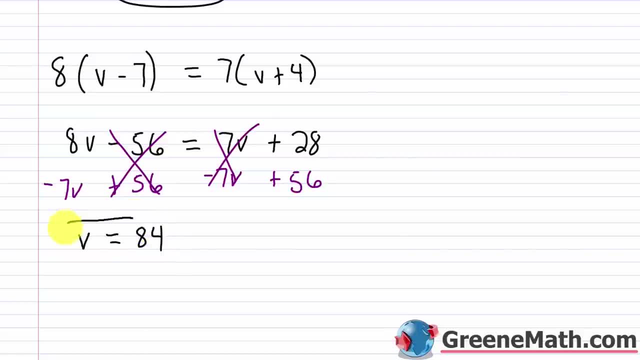 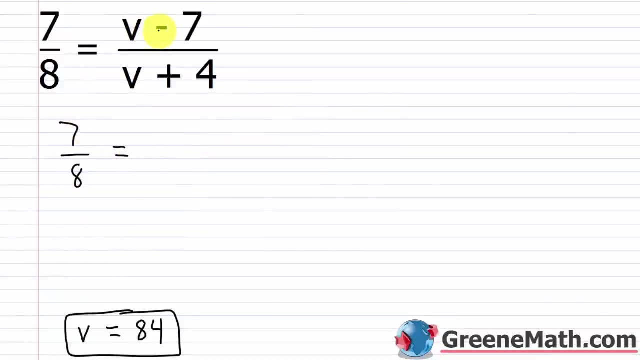 which is 84.. Okay, so v equals 84. is our solution here? All right, so we have 7. eighths is equal to v minus 7. And again, v is going to be 84. So 84 minus 7 over v plus 4.. So again. 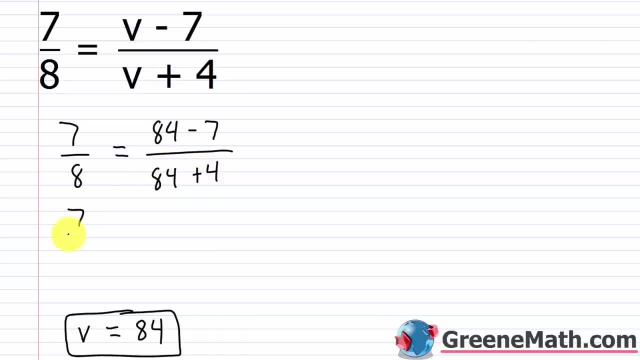 84 plus 7.. And so we'll have 7 eighths over here. What is 84 minus 7?? Well, that's going to be 77.. What is 84 plus 4? That's going to be 88. So each here is divisible by 11.. If I divide 77 by 11,, 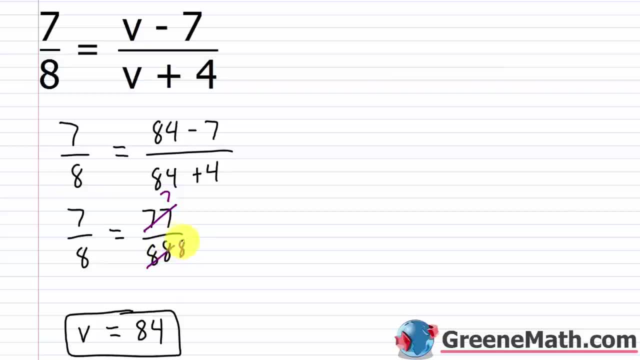 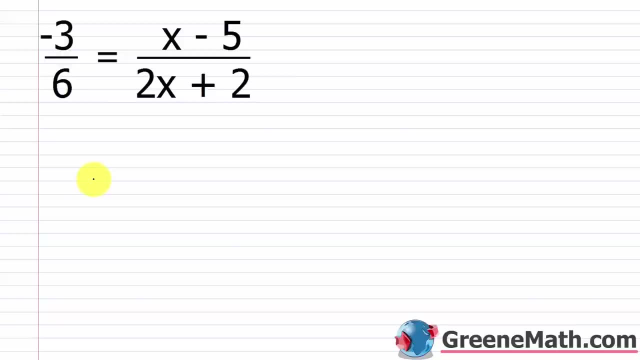 I get 7.. If I divide 88 by 11,, I get 8.. So 7 eighths equals 7 eighths, And so v equals 84 is the correct solution. All right, let's take a look at another one. We have negative 36 equals. x minus 5 over 2x plus 2.. And so we have negative 36 equals x minus 5 over 2x plus 2.. And so we have negative 36 equals x minus 5 over 2x plus 2.. And so we have negative 36 equals x minus 5 over 2x plus 2.. 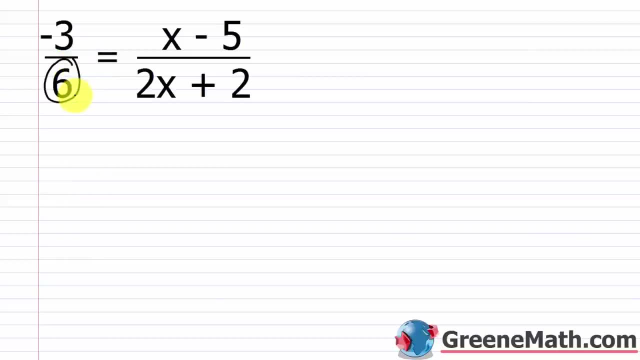 So again I'm going to set up my equation. So 6 is going to be multiplied by this quantity x minus 5.. Again, you have to use parentheses. So 6 times the quantity x minus 5.. This is equal to: 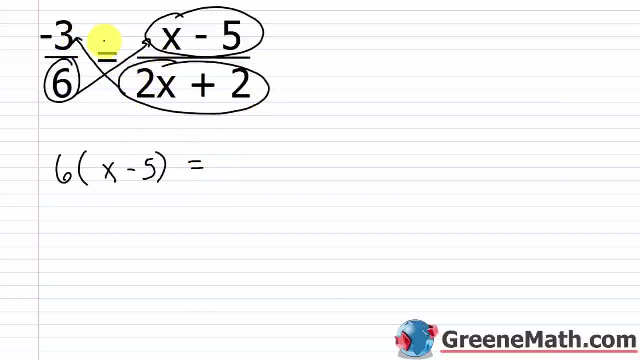 now I'm going to take 2x plus 2, multiply it by negative 3. Okay, so negative 3 times this quantity, 2x plus 2.. Again, you have to use parentheses. You might want to like put that next. 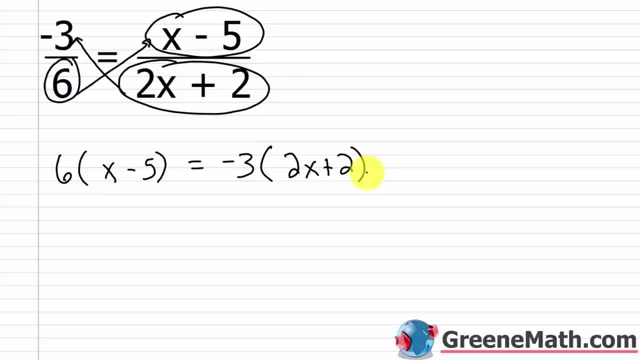 problem like a big star, so that it just gets into your head that I have to use parentheses when I'm multiplying a single number times a quantity. So 6 times x is 6x. then minus 6 times 5, that's 30. This equals negative 3 times 2x. that's negative 6x, then negative 3 times 2 would. 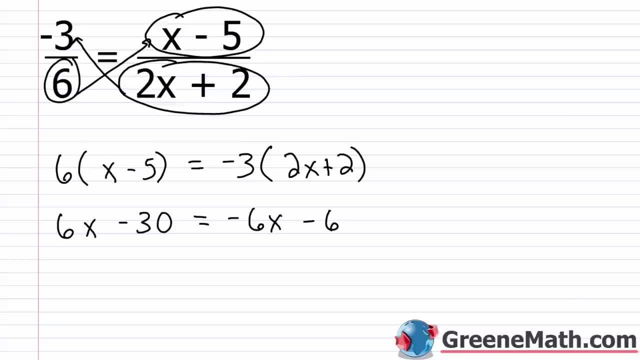 be minus 6.. All right, so I am going to add 6x to both sides of the equation, and I'm also going to add 30 to both sides of the equation. So this will go away, and so will this, and what will I have left? 6x plus 6x is 12x. 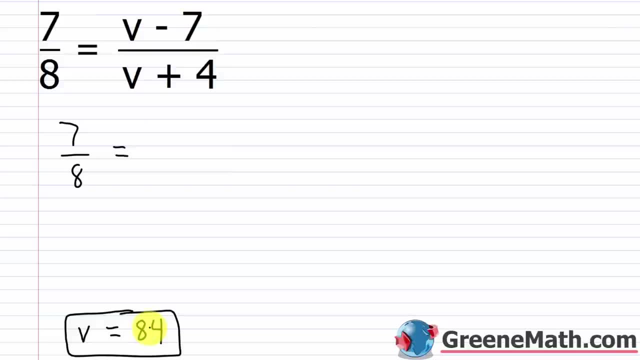 7 eighths is equal to v minus 7. And again, v is going to be 84. So, 84 minus 7 over 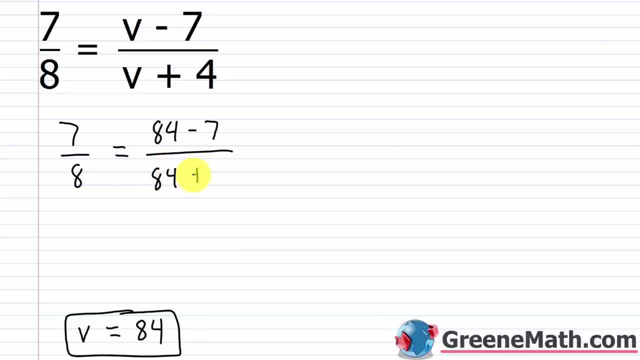 v plus 4. So, again, 84 plus 4. 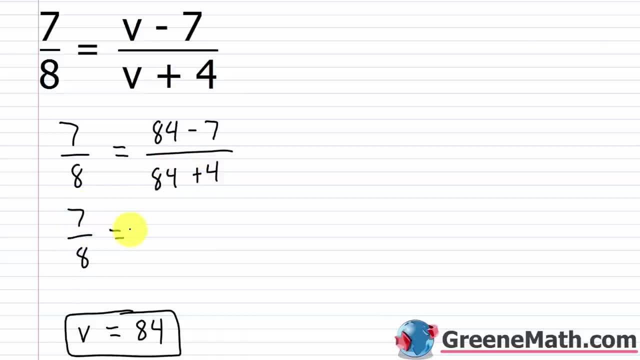 And so, we'll have 7 eighths over here. What is 84 minus 7? Well, that's going to be 77. 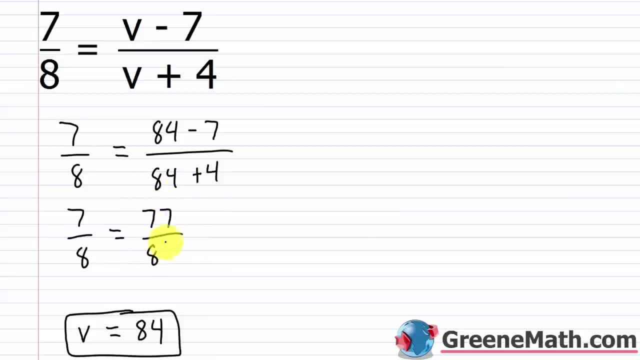 What is 84 plus 4? That's going to be 88. 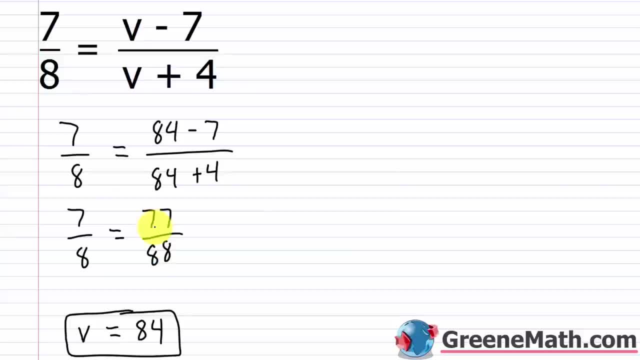 So, each here is divisible by 11. If I divide 77 by 11, I get 7. If I divide 88 by 11, I get 8. 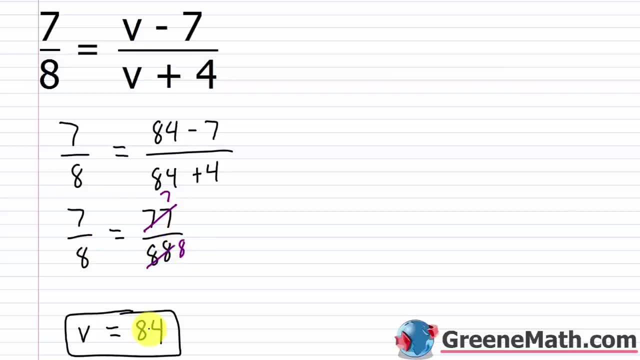 So, 7 eighths equals 7 eighths. And so, v equals 84 is the correct solution. Alright, let's take a look at another one. 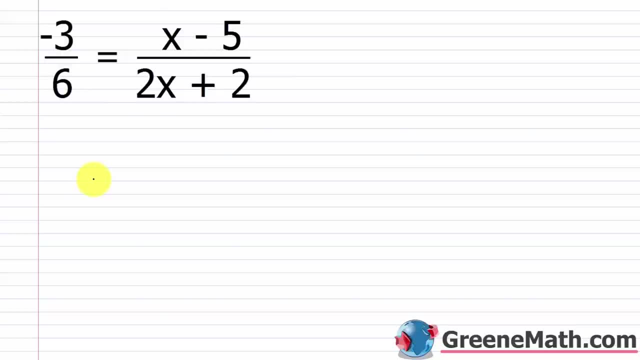 We have negative 36 equals x minus 5 over 2x plus 2. 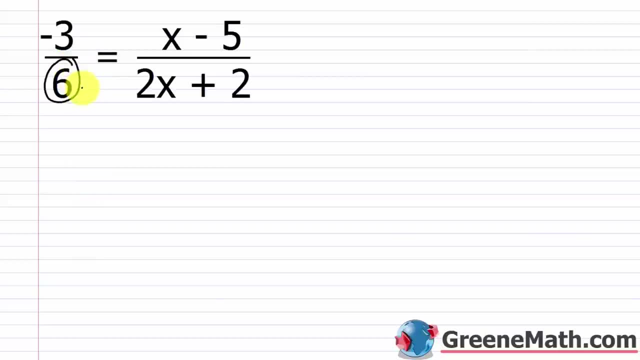 So, again, I'm going to set up my equation. So, 6 is going to be multiplied by this quantity, x minus 5. Again, you have to use parentheses. 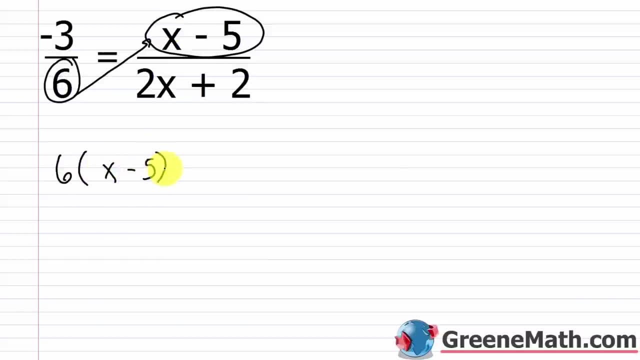 So, 6 times the quantity x minus 5. 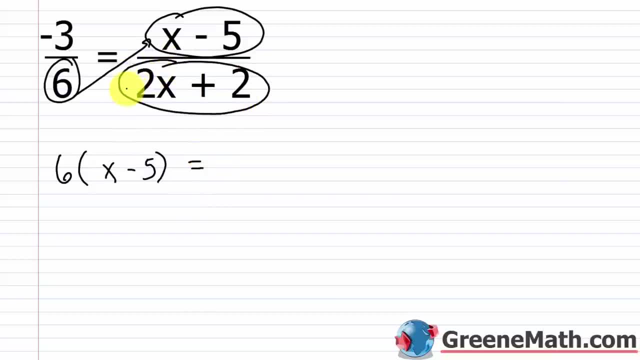 This is equal to, now I'm going to take 2x plus 2, multiply it by negative 3. Okay? 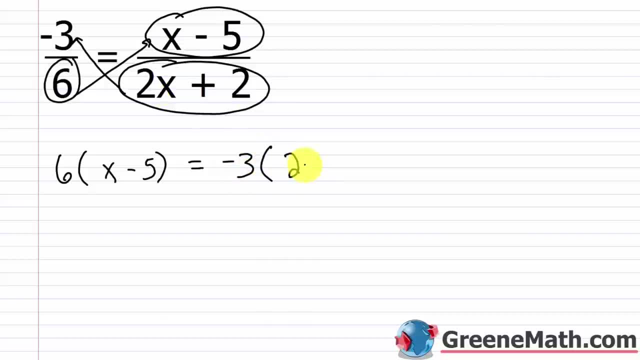 So, negative 3 times this quantity, 2x 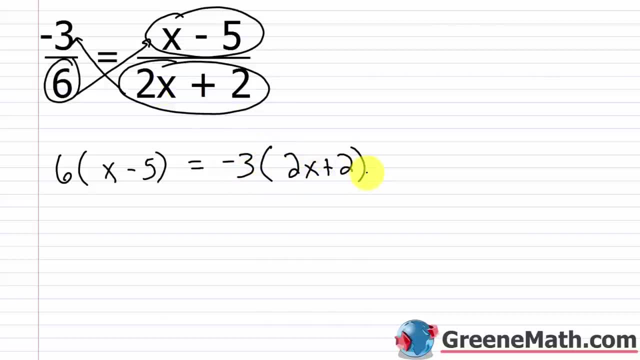 plus 2. Again, you have to use parentheses. You might want to like put that next to each problem 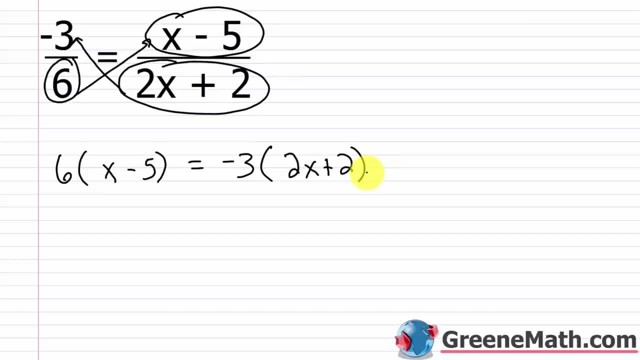 like a big star, so that it just gets into your head that I have to use parentheses when I'm multiplying a single number times a quantity. So, 6 times x is 6x. 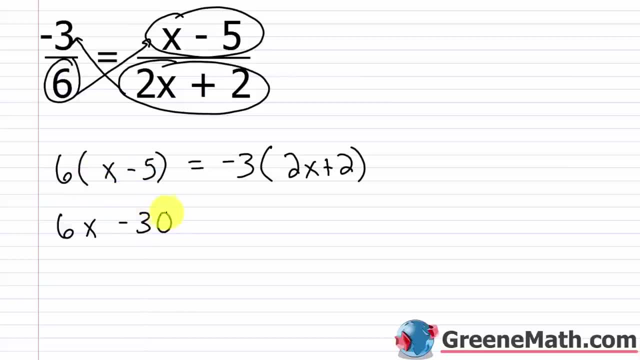 Then minus 6 times 5, that's 30. This equals negative 3 times 2x, that's negative 6x. 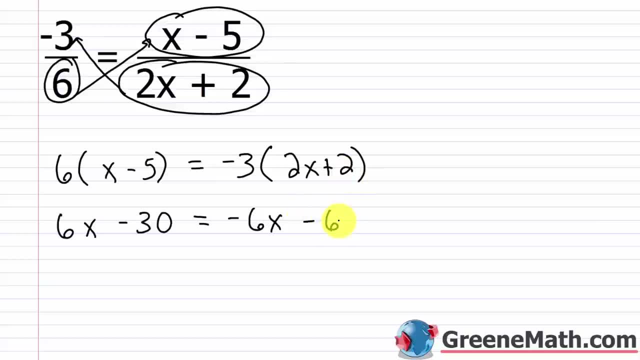 Then negative 3 times 2 would be minus 6. 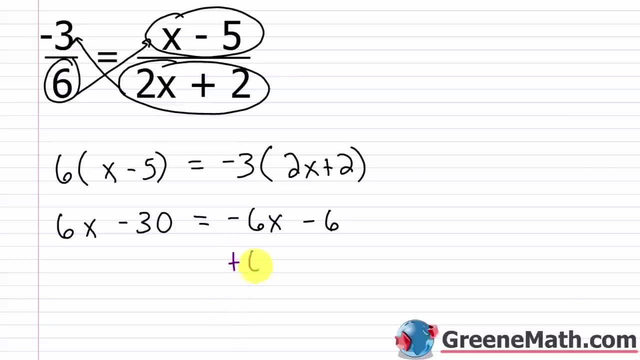 Alright. So, I am going to add 6x to both sides of the equation. 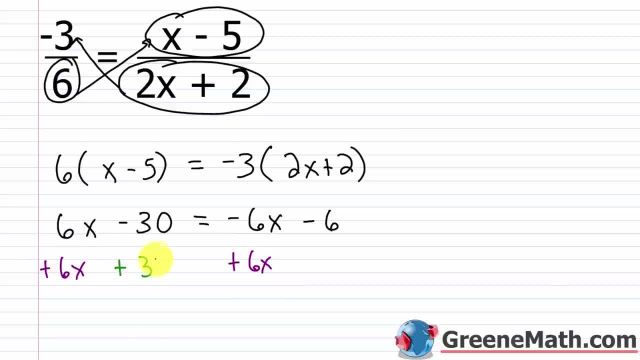 And I'm also going to add 30 to both sides of the equation. 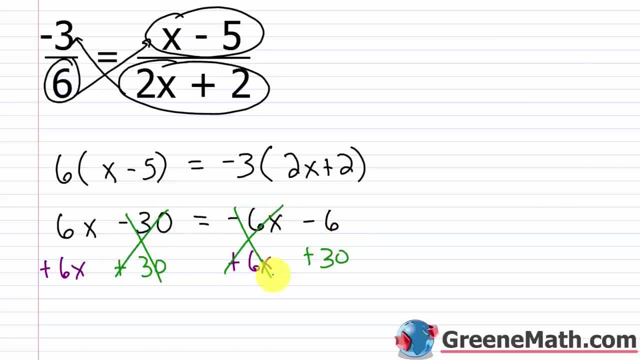 So, this will go away, and so will this. And what will I have left? 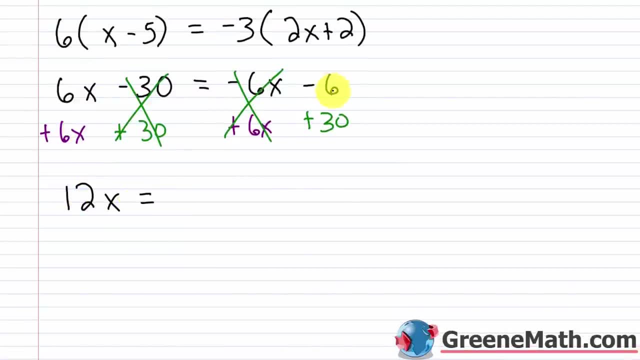 6x plus 6x is 12x. Negative 6 plus 30 is 24. Divide both sides of the equation by 12, the coefficient of x. And we get x is equal to, 24 divided by 12 is 2. 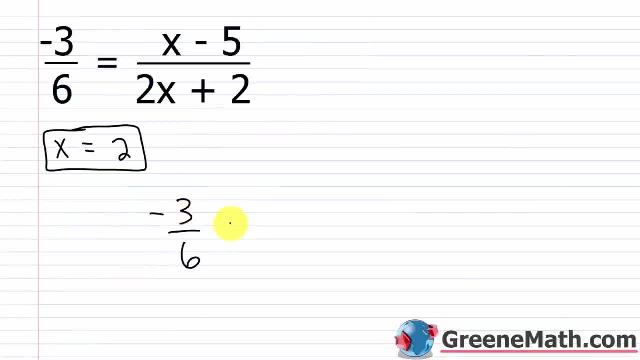 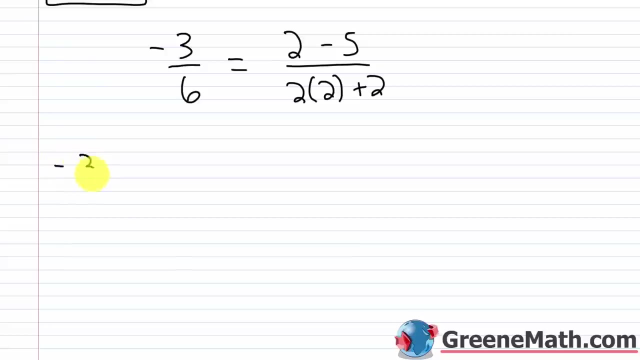 So, we have negative 3 over 6 is equal to, up here I'm going to plug a 2 in for x. So, I'd have 2 and then minus 5 up here. And then down here I'd have 2 times x, so 2 times 2. And then plus 2. So, I'd have negative 3 over 6 is equal to, 2 minus 5 is negative 3. 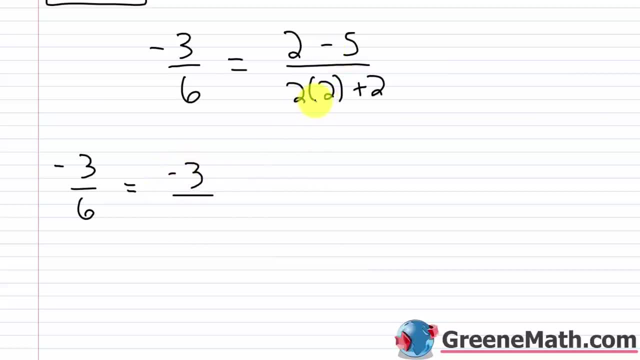 Then 2 times 2 is 4, plus 2 is 6. 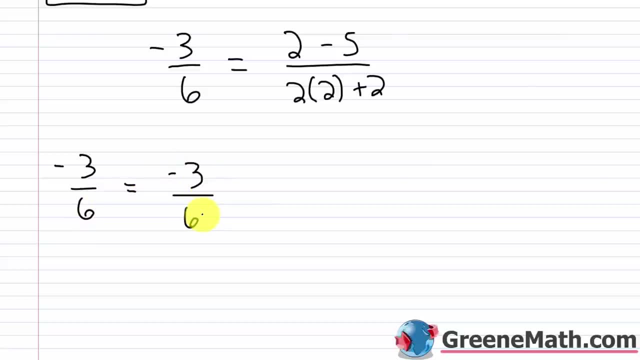 So, we get negative 3 over 6 equals negative 3 over 6. 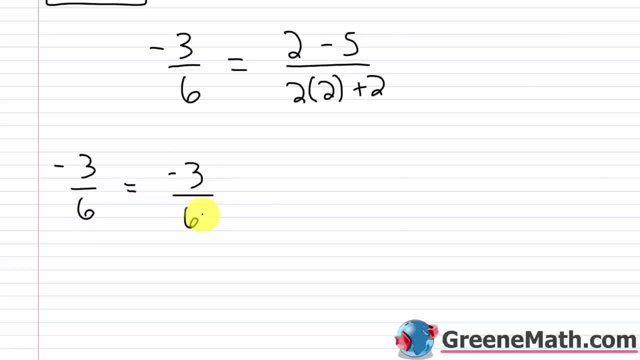 If we wanted to, we could reduce this to negative 1 half in each case. This would divide by 3 and become 1. This would divide by 3 and become 2. Same thing over here. 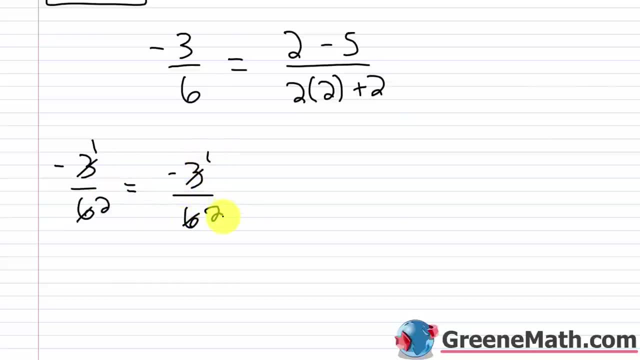 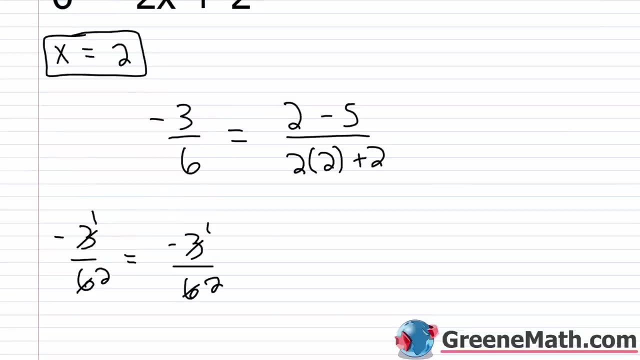 So, we could have negative 1 half equals negative 1 half. But, you could also leave it as negative 3 6 equals negative 3 6. The main point is that your solution here, which was x equals 2, 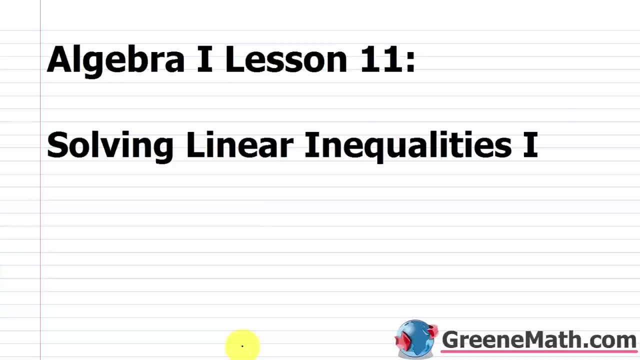 Hello, and welcome to Algebra 1 Lesson 11. In this video, we're going to start talking about how to solve linear inequalities. 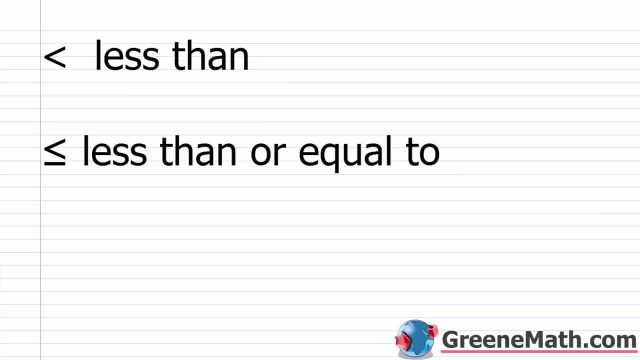 So, this lesson is going to be all about learning how to solve a linear inequality in one variable. Now, the procedure is basically the same as with solving a linear equation in one variable, but with a few key differences. 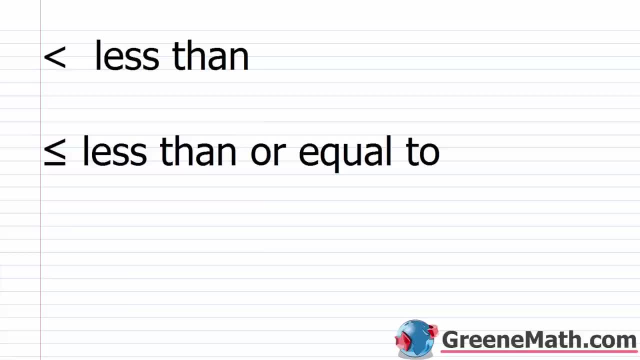 So, let's start out today by just reviewing some basics about inequalities. 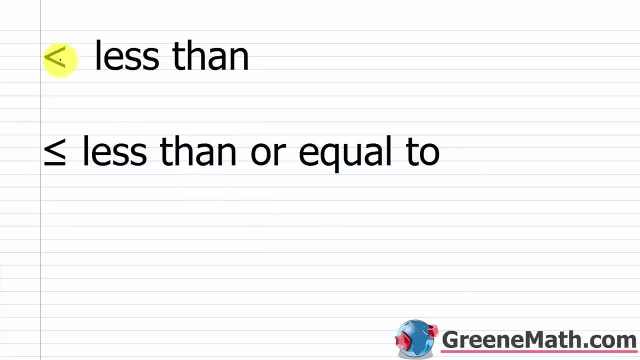 So, the first thing is that this symbol right here, it points to the left. It's known as the less than symbol. 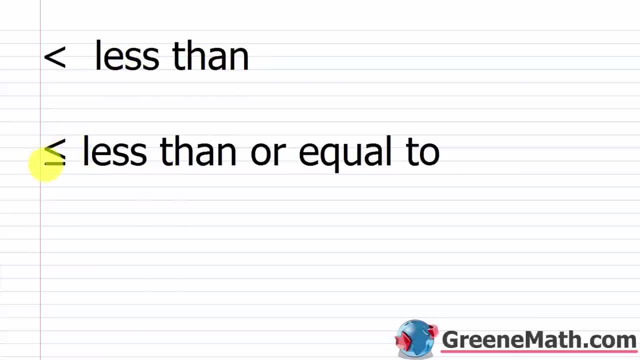 Then, this symbol right here that points to the left with a bar underneath it is the less than or equal to. 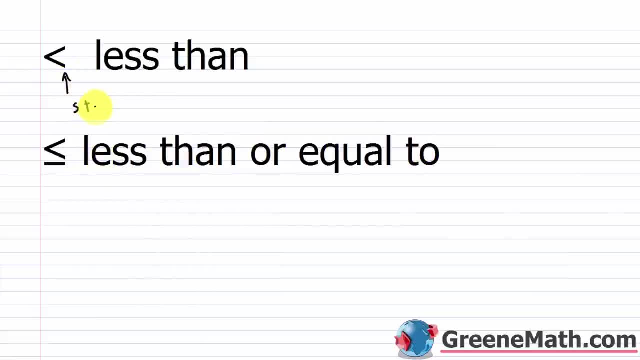 This type of inequality is known as a strict inequality. 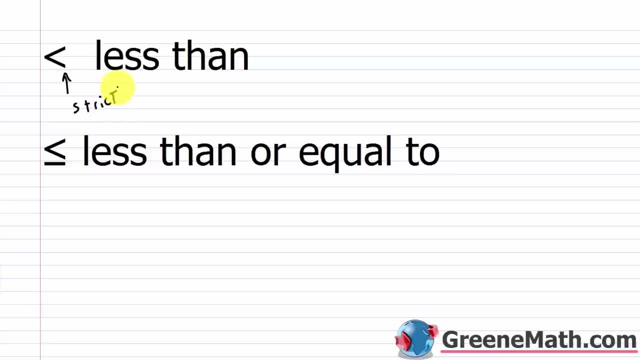 So, something is strictly less than. 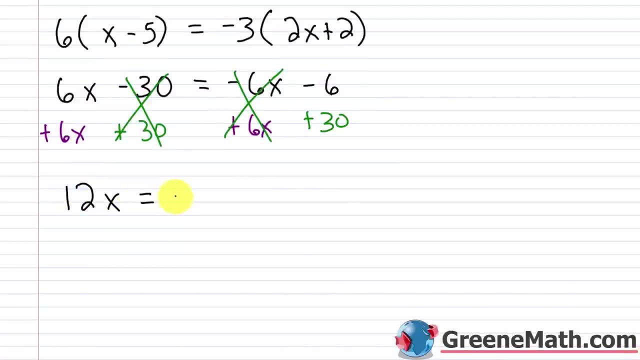 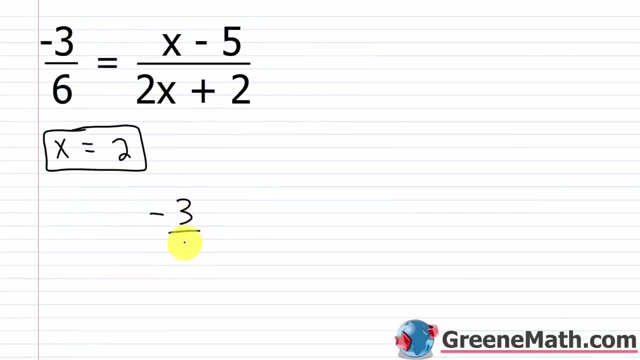 negative 6 plus 30 is 24.. Divide both sides of the equation by 12, the coefficient of x and we get x is equal to 24. divided by 12 is 2.. So we have negative. 3 over 6 is equal to up here I'm going to plug a 2 in for x, so I'd have 2. 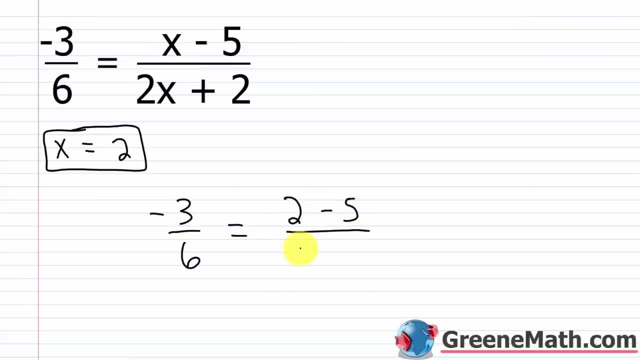 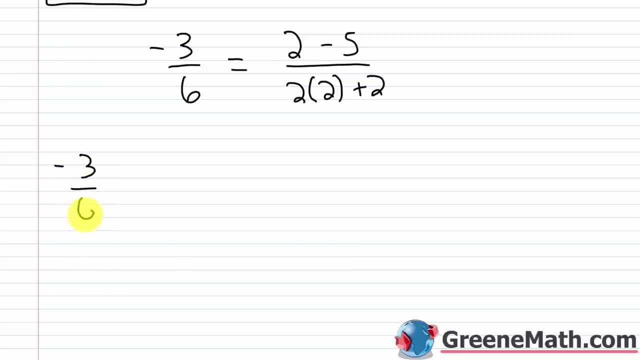 and then minus 5 up here and then down here. I'd have 2 times x, so 2 times 2 and then plus 2.. So I'd have negative 3 over 6 is equal to 2, minus 5 is negative 3. 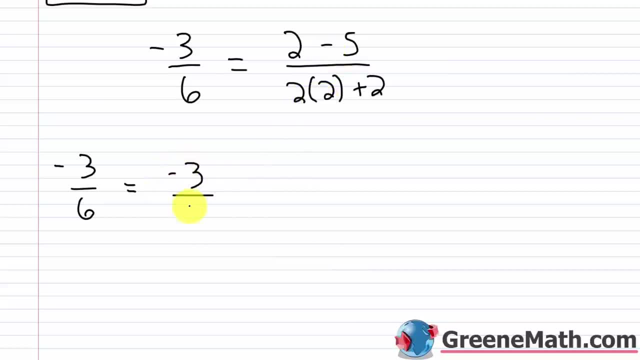 then 2 times 2 is 4 plus 2 is 6.. So we get negative 3 over 6 equals negative 3 over 6, and if we wanted to, we could reduce this to negative one half in each case. right, this would divide by: 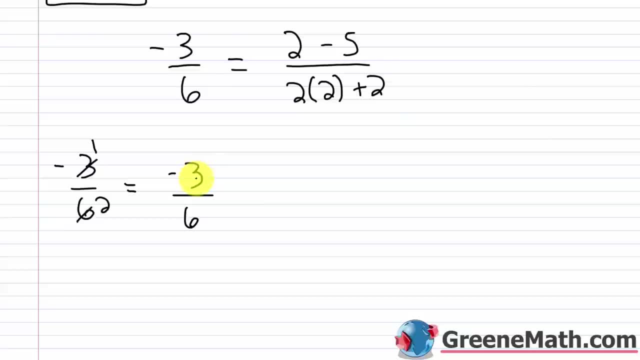 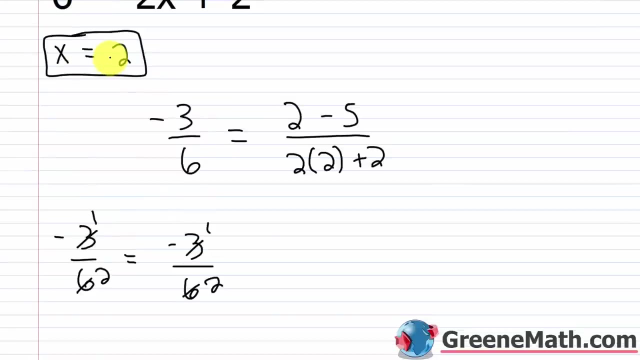 3 and become 1. this would divide by 3 and become 2. same thing over here. So we could have negative one half equals negative one half, but you could also leave it as negative 3 6 equals negative 3, 6. the main point is that your solution here, which was x equals 2, is correct. 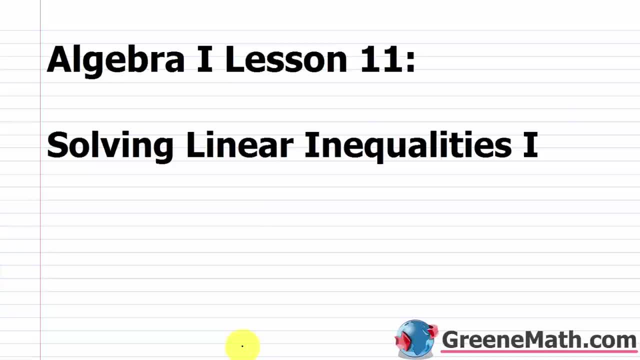 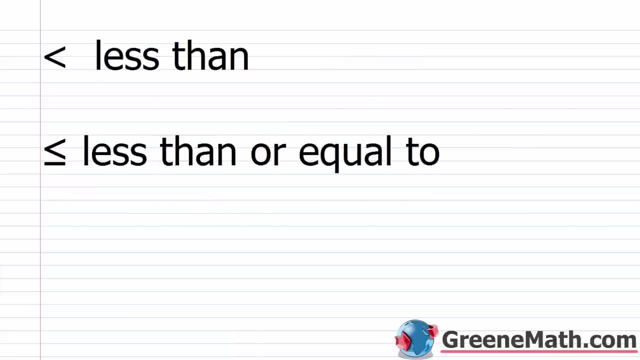 Hello and welcome to algebra 1, lesson 11.. In this video, we're going to start talking about how to solve linear inequalities. So this lesson is going to be all about learning how to solve a linear inequality in one variable. Now the procedure is basically the same as with solving 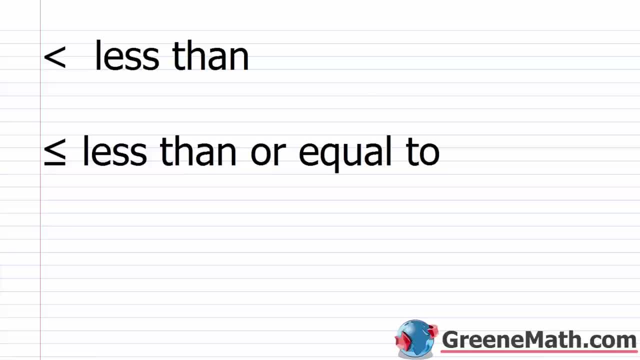 a linear equation in one variable, but with a few key differences. So let's start out today by just reviewing some basics about inequalities. So the first thing is that this symbol right here it points to the left. it's known as the less than symbol. Then this symbol right here, that's: 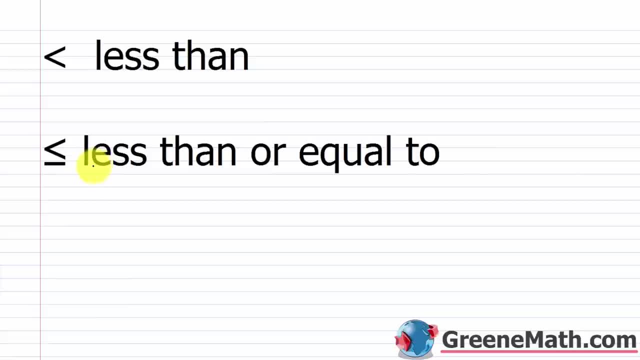 points to the left with a bar underneath. it is the less than or equal to. This type of inequality is known as a strict inequality, So something is strictly less than. This type of inequality is known as a non-strict. a non-strict inequality, So it allows for the possibility that they're 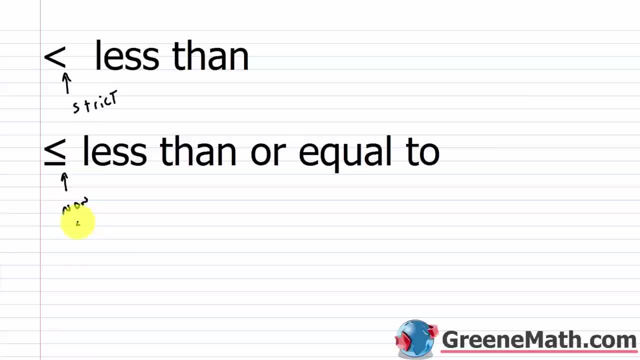 This type of inequality is known as a non-strict. A non-strict inequality. 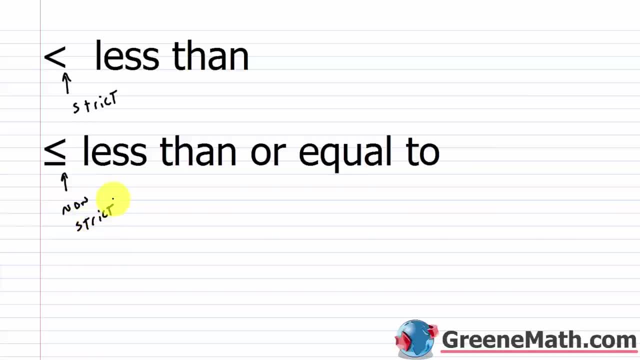 So, it allows for the possibility that they're equal. 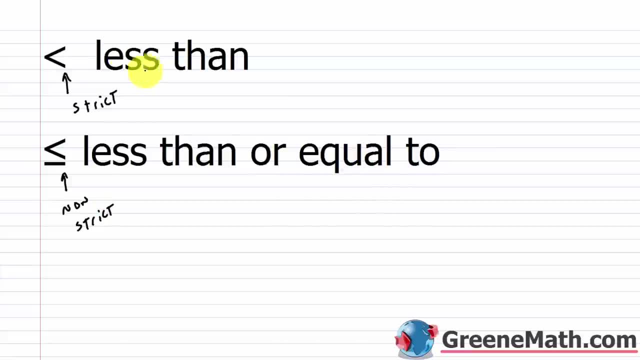 It says or equal to. In this case, it's strictly less than. In this case, it's less than 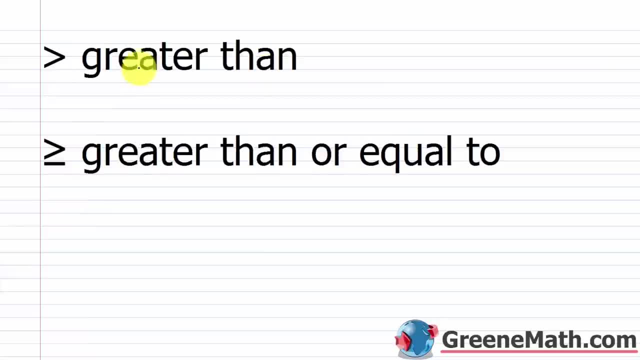 or equal to. Now, we also have the greater than. This points to the right. Then, we have the greater than or equal to. It points to the right, but has a bar underneath it. And again, this greater than is a strict inequality. This is a strict inequality. 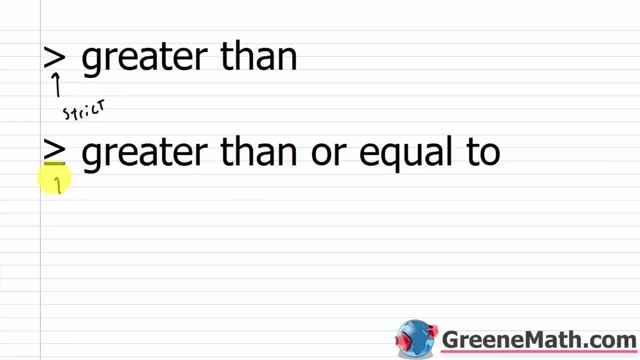 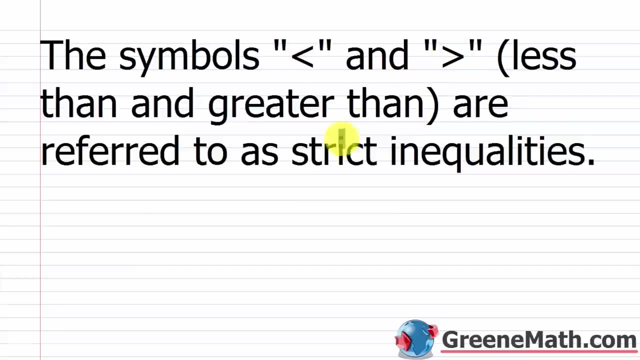 Strictly greater than. This type of inequality, this greater than or equal to, is a non-strict. That's because we allow for this or equal to. So, again, the symbols less than and greater than are referred to as strict, strict inequalities. 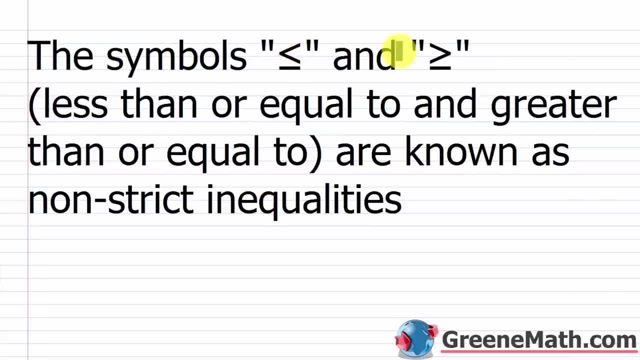 Then, the symbols less than or equal to and greater than or equal to are known as non-strict inequalities. 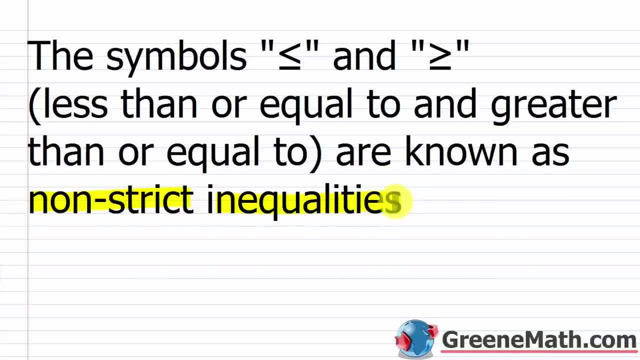 Very important that you understand the difference between the two. So, in order to start thinking about inequalities 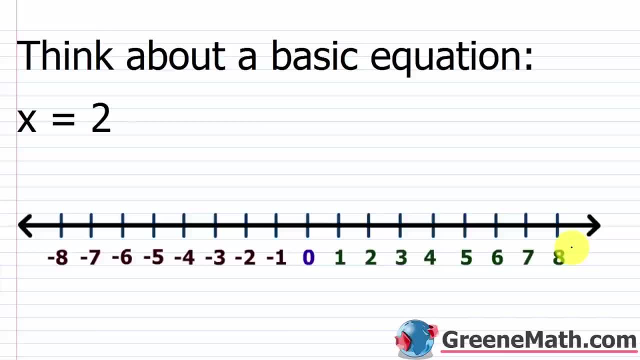 in the right way, I want you to first think about a basic equation. 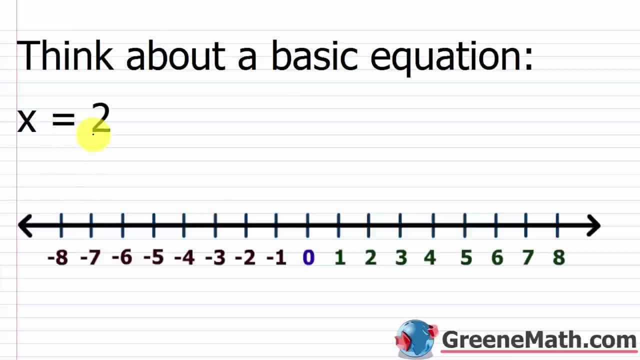 Let's say we have something like x equals 2. So, if I was to graph x equals 2 using this basic number line, what I would do is I would take and I would put a filled in dot or filled in circle, however you want to think about that, specifically at the number 2 on the number line. 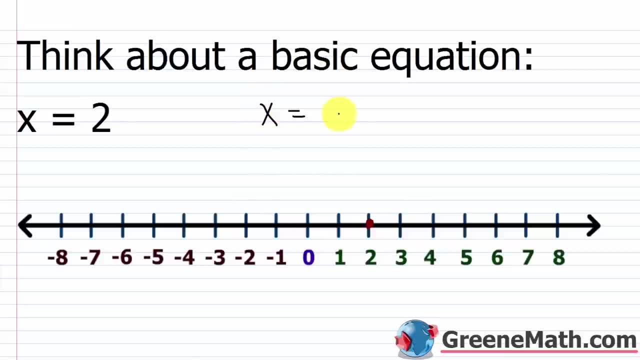 If I had something different, let's say I had x equals 5, for example. Let me do this in a different color so that we don't get confused. So, let's say I had x equals 5. Well, I would graph that by putting a filled in dot or a filled in circle at 5. That's my solution. 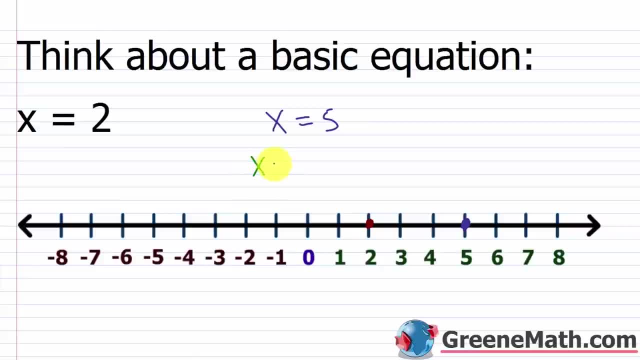 Let's look at one more. Let's say we had x equals negative 3. Well, I'd put in, again, a filled in dot or a filled in circle at negative 3. So, in each case, we're showing a visual representation of the solution to the equation. And this is going to get much more complex as we go throughout algebra, but right now this is about as basic as it gets. 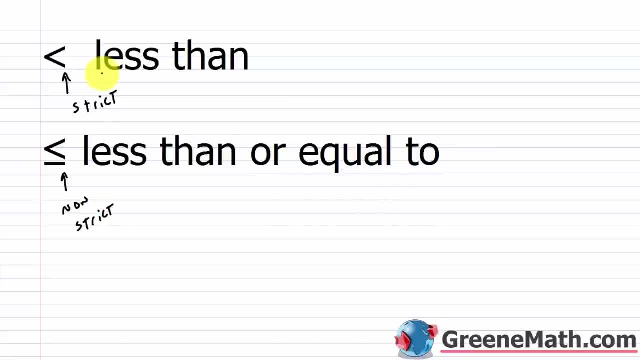 equal right, it says: or equal to right. in this case it's strictly less than. in this case it's less than or equal to. Now we also have the greater than. this points to the right. and then we have the greater than or equal to points to the right, but has a bar underneath it, and again this: 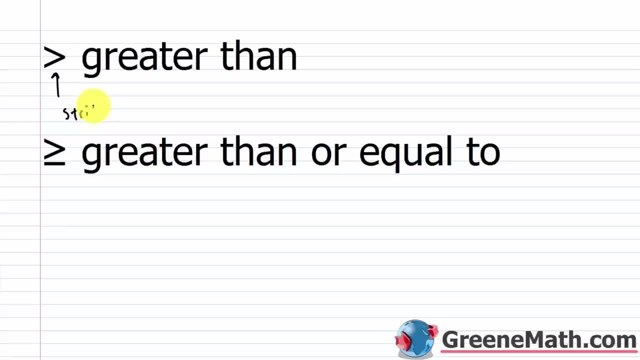 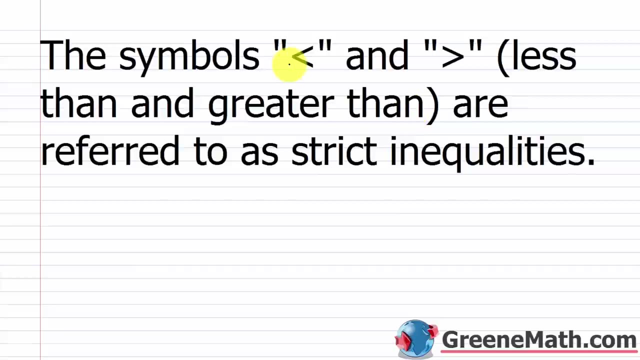 greater than is a strict inequality. This is a strict inequality, strictly greater than This type of inequality. this greater than or equal to is a non-strict, is a non-strict. That's because we allow for this or equal to. So again, the symbols. 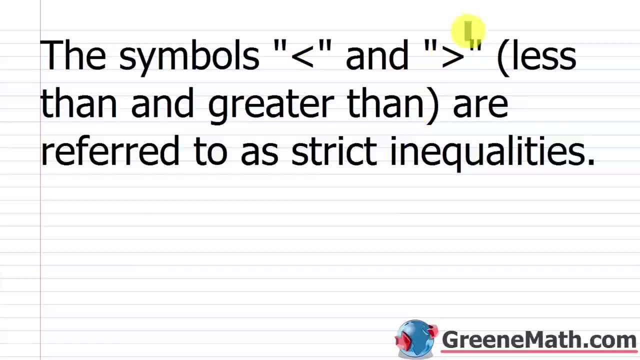 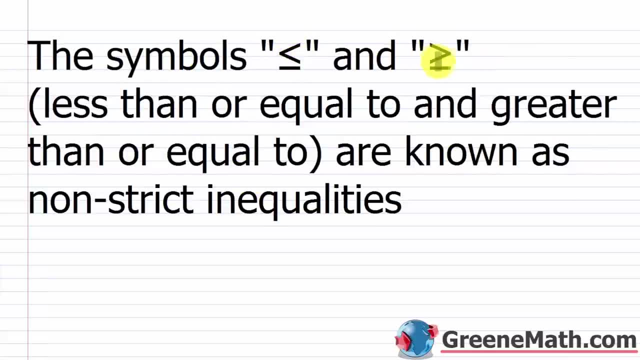 less than and greater than are referred to as strict, strict inequalities. Then the symbols less than or equal to, and greater than or equal to are known as non-strict inequalities. Very important that you understand the difference between the two. So, in order to start thinking about, 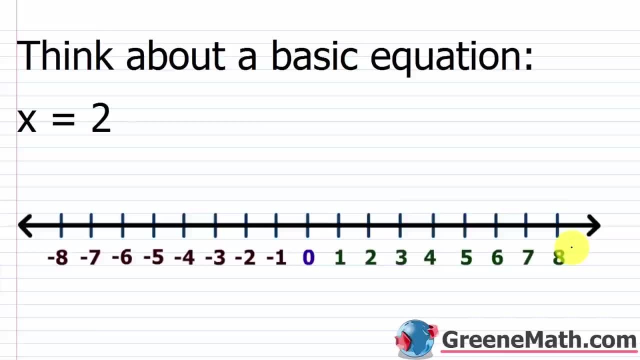 inequalities in the right way. I want you to first think about a basic equation. Let's say we have something like x equals two. So if I was to graph x equals two using this basic number line, what I would do is I would take and I would put a filled in dot or filled in circle. 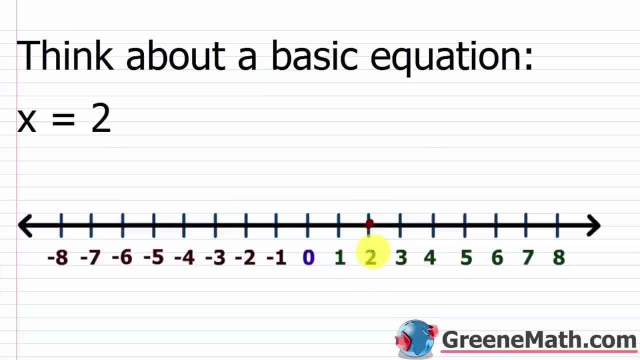 however, you want to think about that specifically at the number two on the number line. If I had something different- let's say I had x equals five, for example, Let me do this in a different color so that we don't get confused. So let's say I had x equals five, Well, I would graph that by putting: 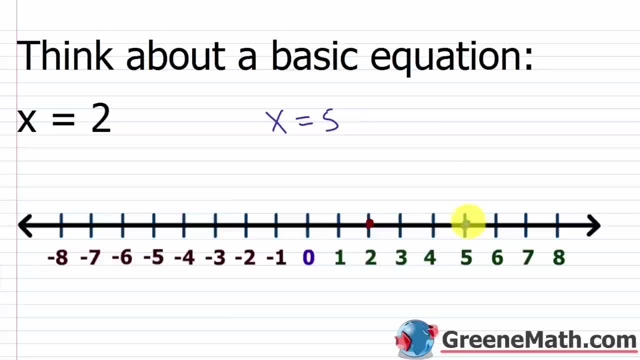 a filled in dot or a filled in circle at five. That's my solution. Let's look at one more. Let's say we had x equals negative three. Well, I'd put in again a filled in dot or filled in circle at negative three. So in each case we're showing a visual representation. 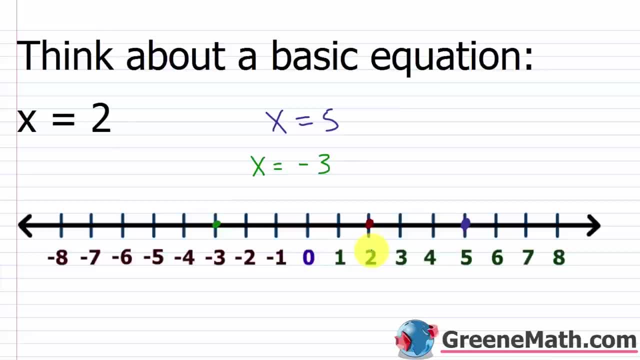 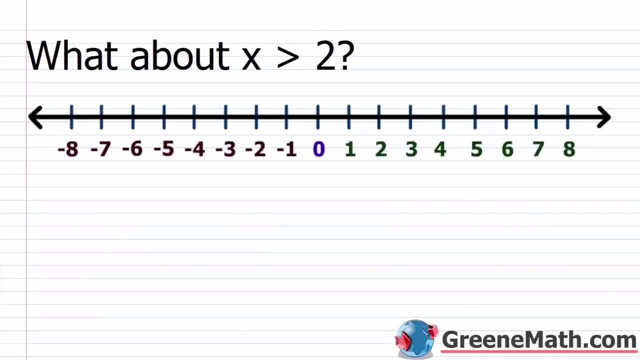 of the solution to the equation, and this is going to get much more complex as we go throughout algebra. For right now, this is about as basic as it gets. What about? x is greater than two? How would I graph that? Well, we're going to come back to this, but I just want you to realize that, in the case of an equation, 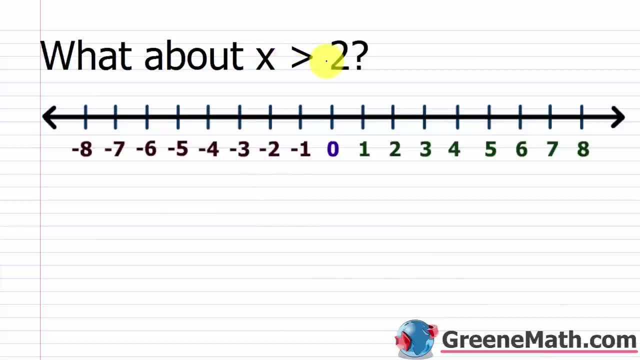 What about x is greater than 2? How would I graph that? 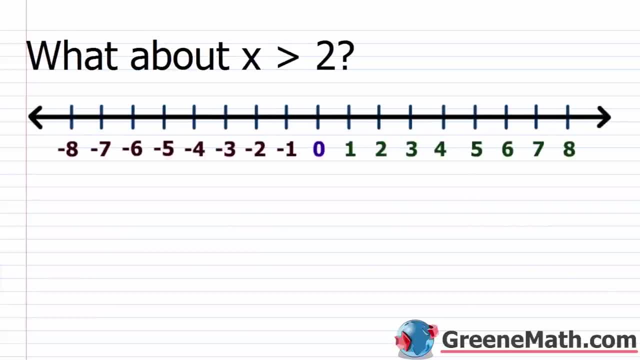 Well, we're going to come back to this, but I just want you to realize that in the case of an equation, we have an exact number. It's kind of a laser focus. It's x has to be 2. It's equal to 2. 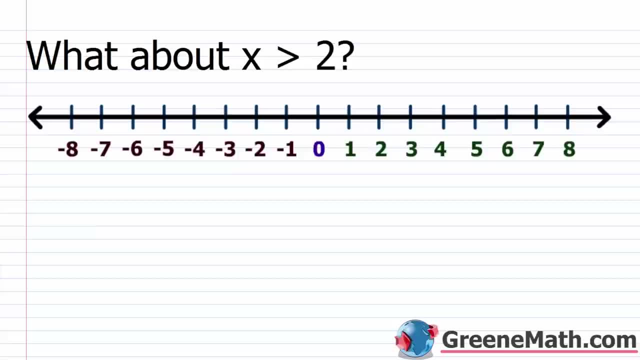 In this case, where we have x is greater than 2, we're now thinking about a range of values, because x can really be anything larger than 2. 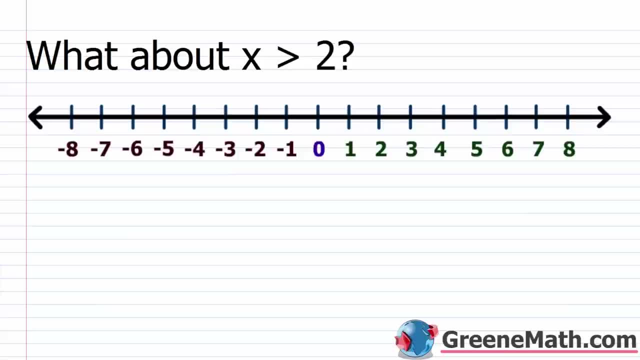 And this is a true statement. If I replaced x with, let's say, 7, and I had 7 is greater than 2, this is true. Right? This is true, because this 7 is 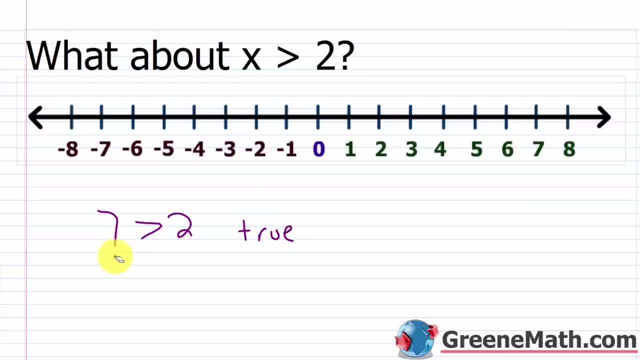 greater than this number 2. So that's true. If I put something in that's 2 or lower than 2, it's going to be false. So, like, 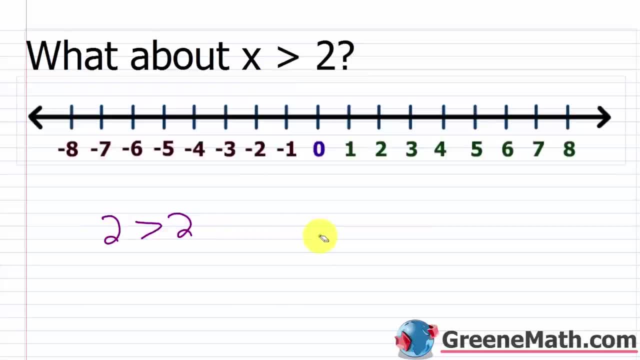 for example, if I put in 2, that's false. 2 is not greater than 2. 2 is equal to 2. So this is false. Or if I put something much lower than 2, let's say, I don't know, negative 7. Negative 7 is not greater than 2. Again, this is false. So 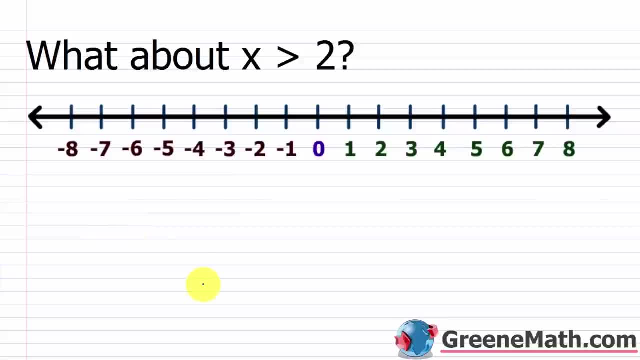 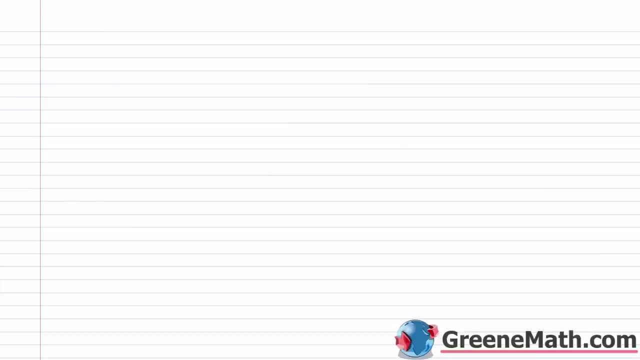 when we think about inequalities, our solution is generally going to be a range of values. So in order to deal with that, we have something known as interval notation. Let me just write that down. We have interval and then notation. 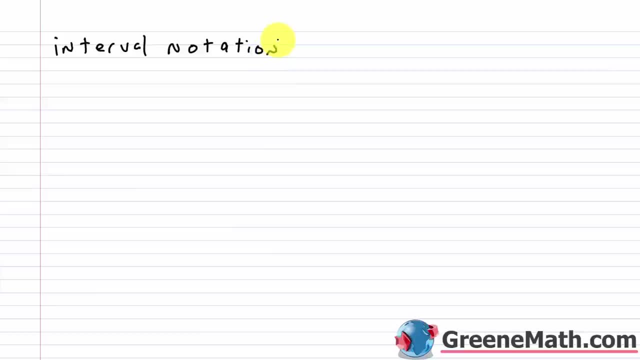 And so this notation is going to specifically help us deal with a solution that's a range of values. Now, typically, the way you're going to write this, you're going to have your smallest value, your smallest value, then comma, your largest, your largest value. 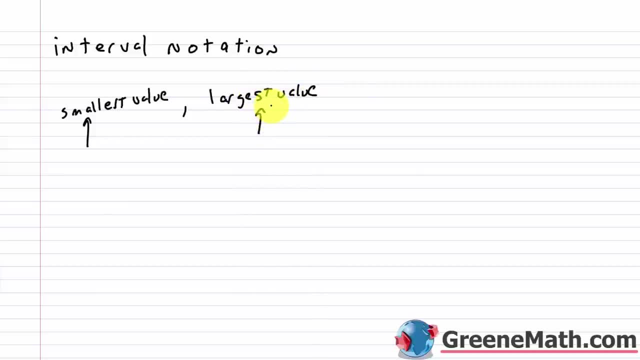 Now, it's not going to exactly work out this way because in a lot of cases, you're going to see you can't exactly put the smallest value because it's impossible for you to list it. So you're going to put something close to that and then you're going to use a special type of notation. So let's kind of jump in and just think about x is greater than 2. 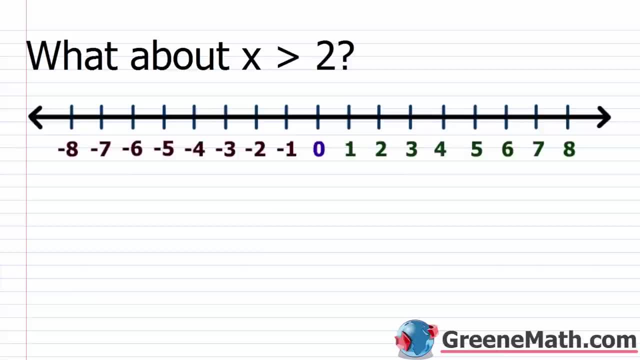 we have an exact number. It's kind of a laser focus. It's: x has to be two, It's equal to two. In this case, where we have x is greater than two, we're now thinking about a range of values, because x can really be anything larger than two, and this is a true statement. If I replaced x with 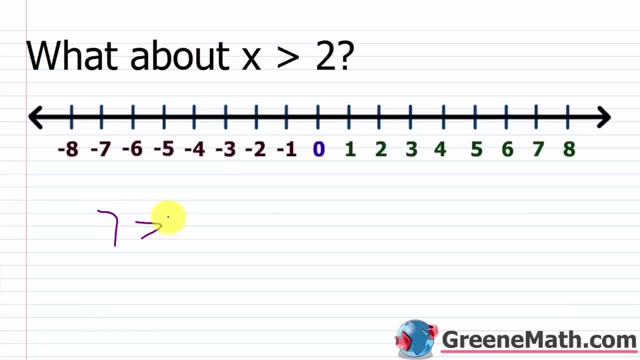 let's say seven and I had seven is greater than two. This is a true statement. If I replaced x with, let's say, seven and I had seven is greater than two, This is true because this seven is greater than this number two. So that's true If I put something. 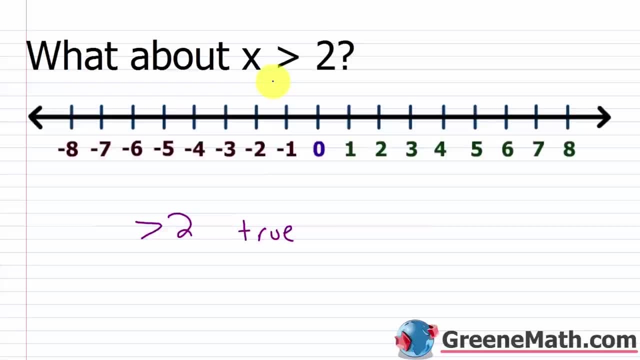 in that's two or lower than two, it's going to be false. So like, for example, if I put in two, that's false. Two is not greater than two. Two is equal to two, So this is false. Or if I put something much lower than two, let's say I don't know- negative seven. Negative seven is not greater. 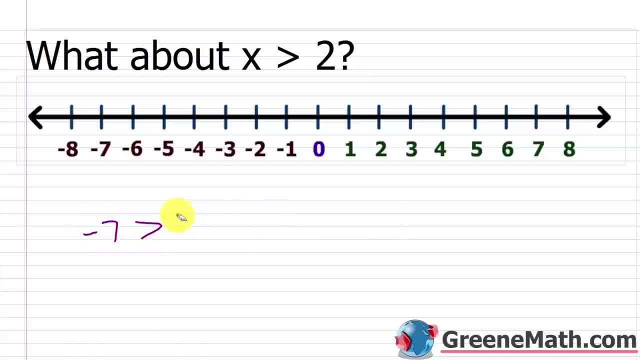 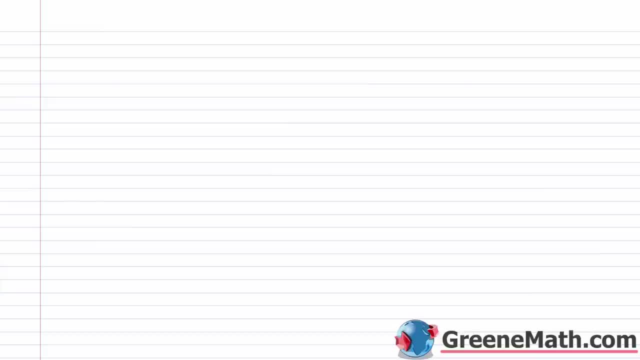 than two. Again, this is false. So, when we think about inequality, This is false. So what are the things that we can do about it? Let's say, we, that's a set of values, and one of these values we could say is one of these and this is our set of values. I know this is false. I have bigger than two. 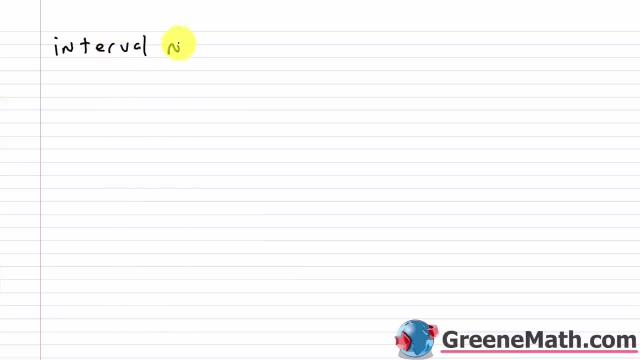 This is just one in this element. but now let's look at something else. just to picture, If we don't have any sub quartiles in a set of values, let's say that we have something greater than the other two of values. now, typically, the way you're gonna write this, you're gonna have your 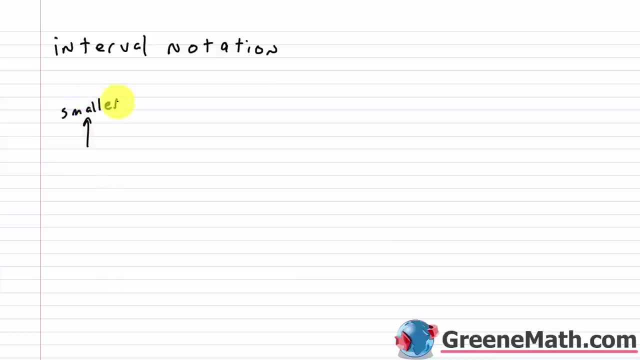 smallest value- your smallest value. then comma: your largest- your largest value. now it's not gonna exactly work out this way because in a lot of cases you're gonna see you can't exactly put the smallest value because it's impossible for you to list it, so you're gonna put something close to that and then you're. 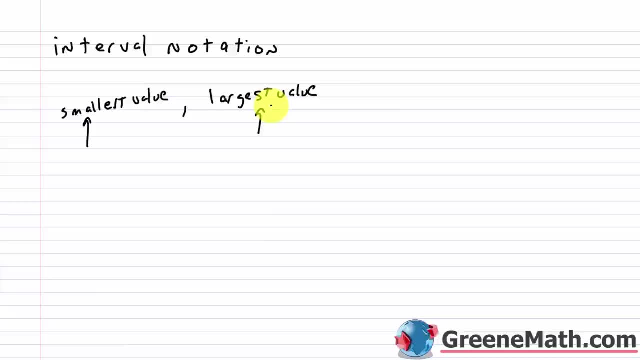 gonna use a special type of notation, so let's kind of jump in and just think about: X is greater than 2. this is what we saw before. if I want to use interval notation, what's the smallest possible value that X can take on? well, it can't. 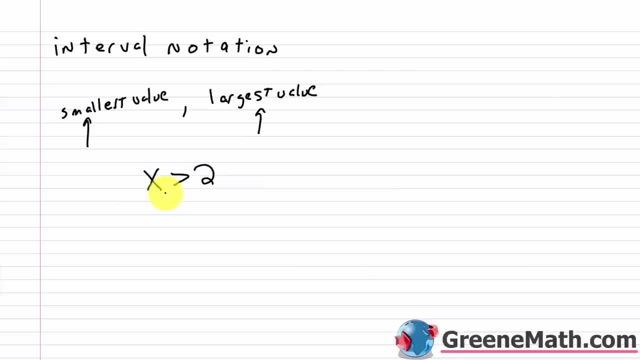 take on 2, but it could be anything larger than 2. if I think about what's the smallest number that you can think of, that's larger than 2. well, you might say, okay, 2.1. and then you could get smaller. you could say, okay, well, 2.1. 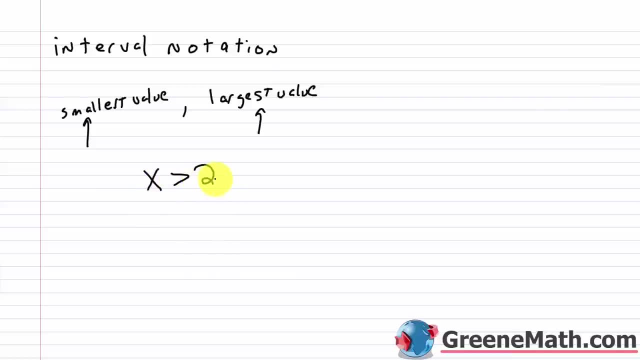 This is what we saw before. If I want to use interval notation, 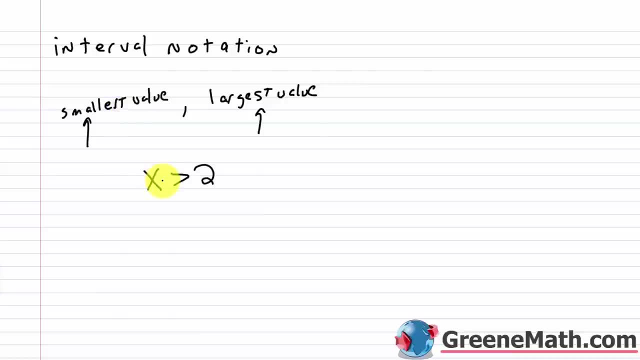 what's the smallest possible value that x can take on? Well, it can't take on 2, but it could be anything larger than 2. If I think about, what's the smallest number that you can think of that's larger than 2? Well, you might say, okay, 2.1. 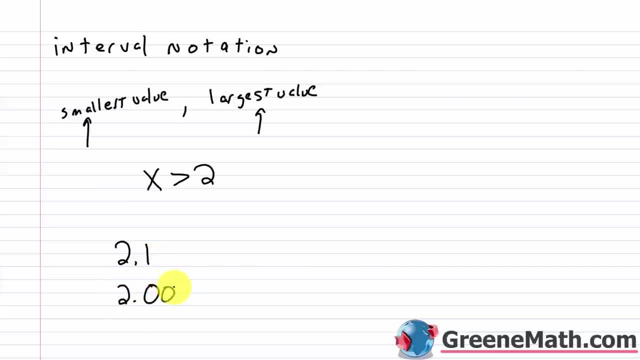 And then you could get smaller. You could say, okay, well, 2.0001. You could get smaller and say 2.00000000001. And you could keep doing that forever and ever and ever. So because you can't possibly list the smallest value that is larger than 2, you're just going to put 2 there. 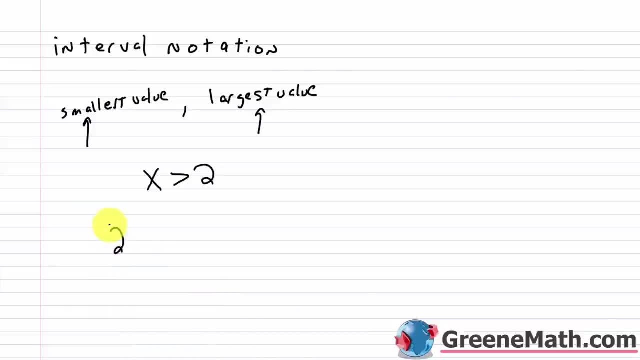 And you're going to place a parenthesis to the left of that to say that the 2 is not included. 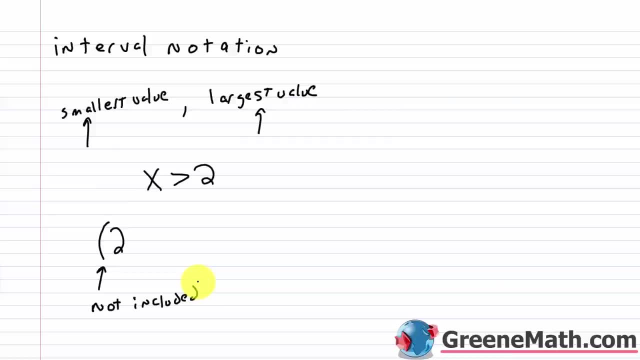 So it's not included in the solution. So when we look at this and we see it, we say, okay, the smallest value is anything larger than 2. 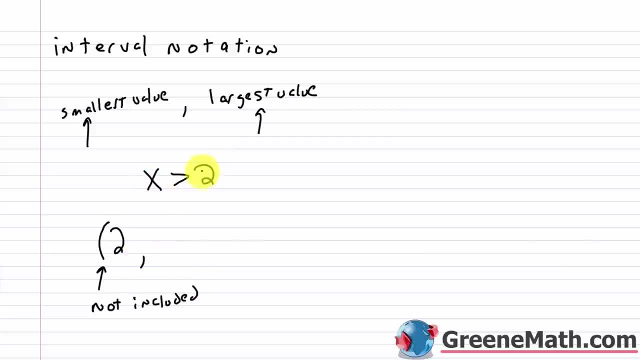 Now, I'm going to put a comma. Now, if x is greater than 2, what's the largest value that x can take on? Well, in terms of numbers, there's really not one because numbers continue forever. So whatever the largest number is that you can think of, you can always add one and get to the next largest. So to kind of notate this concept, we use the infinity symbol. 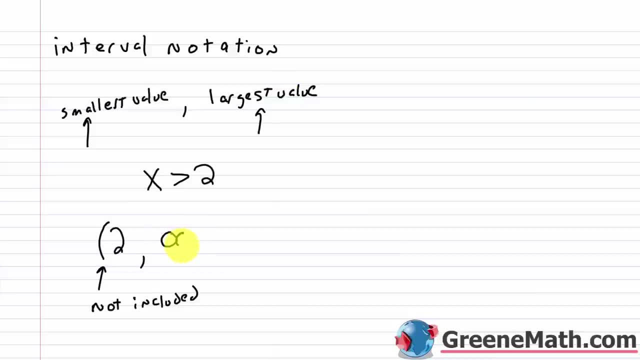 So the infinity symbol. And it kind of looks like a sideways 8. And because infinity is not a number, you're also going to put a parenthesis next to it 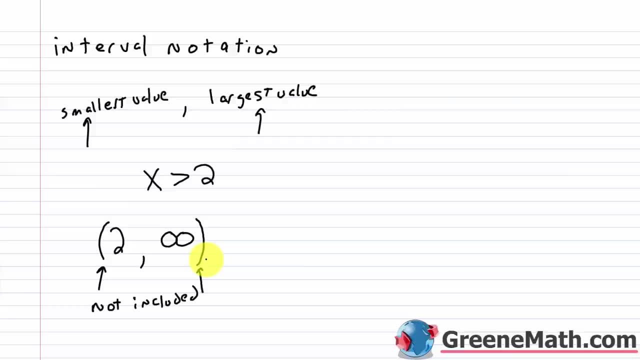 to say that, hey, this is not included. Right? It's not included. 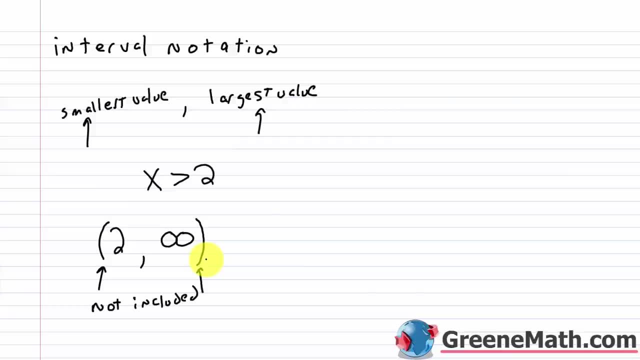 Now, we're going to see in a minute that we're going to have a different type of notation when things are included. 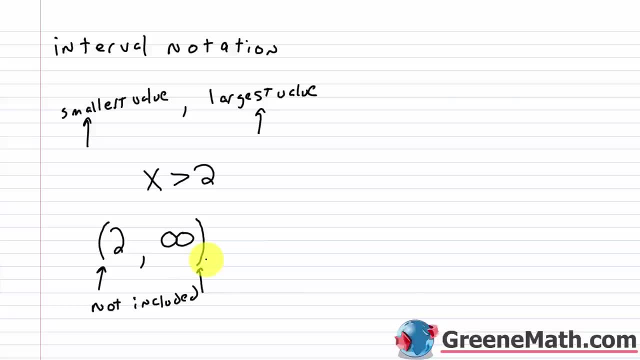 So, we see our interval notation for x is greater than 2. 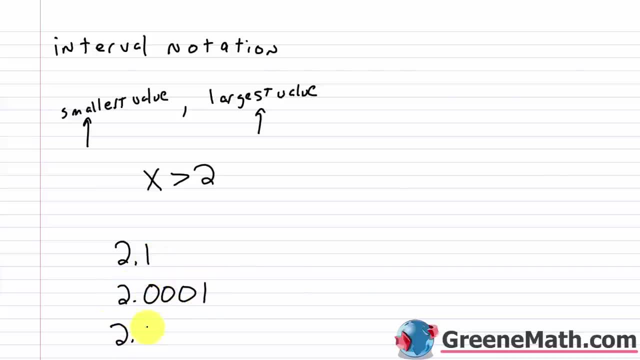 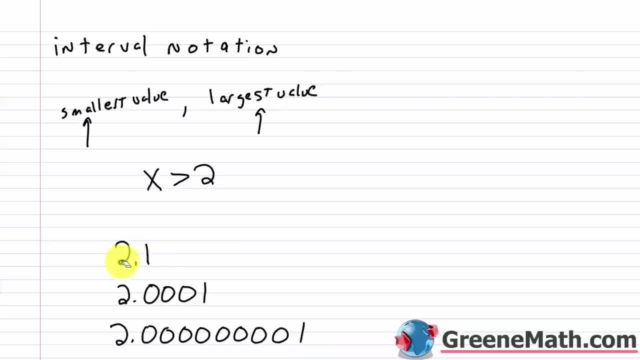 smallest value that is larger than 2. you're just gonna put 2 there and you're going to place a parenthesis to the left of that to say that the 2 is not included. so it's not included in the solution. so when we look at this and we see it, we 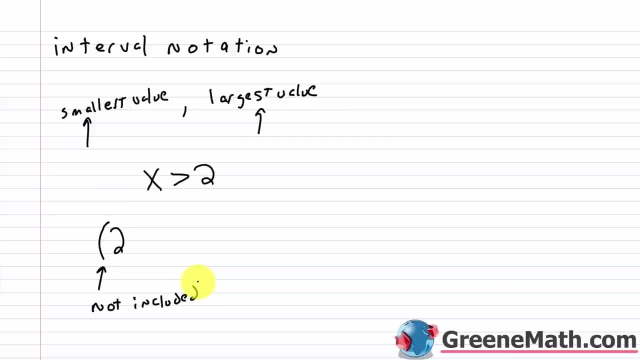 say: okay, the smallest value is anything larger than 2. now I'm gonna put a comma. now, if X is greater than 2, what's the largest value that X can take on? well, in terms of numbers, there's really not one, because numbers continue forever. whatever the largest number is that you can think of, you can always add one and 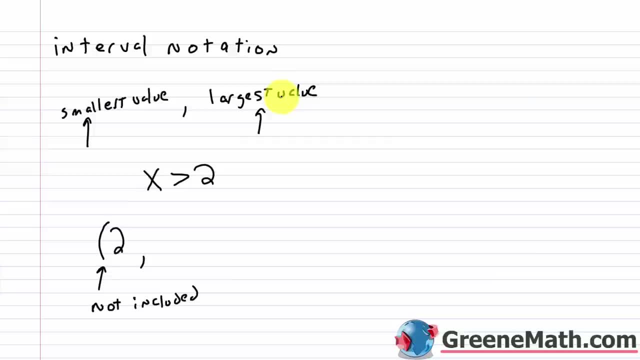 get to the next largest. so to kind of notate this concept, we use the infinity symbol. so the infinity symbol and it kind of looks like a sideways 8, and because infinity is not a number, you're also going to put a parenthesis next to it to say that, hey, this is not included. right, it's not included now. 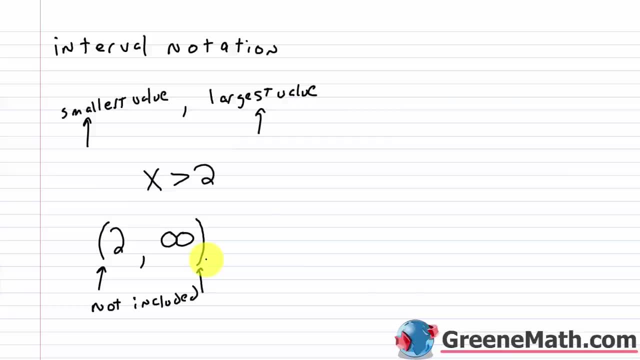 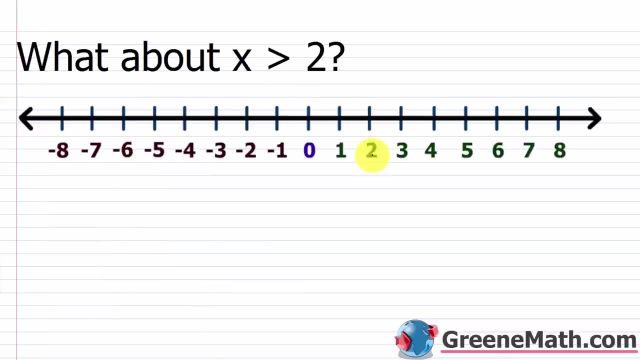 we're gonna see in a minute that we're gonna have a different type of notation when things are included. so we see our interval notation for X is greater than 2. how do we use this to graph? well, it's similar. if I have X is greater than 2, I find 2 on the number line and what I'm gonna do. 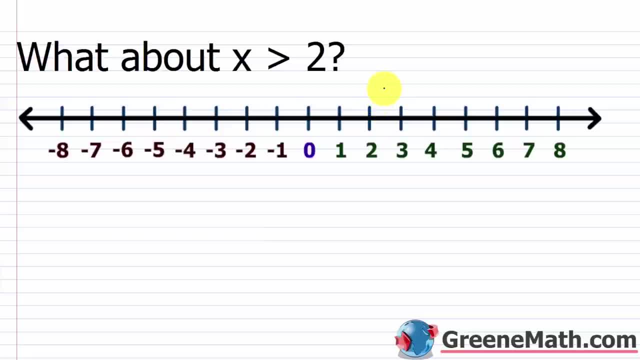 is, I'm gonna put a parenthesis at 2 that faces in the direction of my solution. so this is gonna face to the right, because everything larger than 2 is in the solution. the parenthesis is telling me that 2 is not included. not included, and then I'm gonna shade everything to the right. 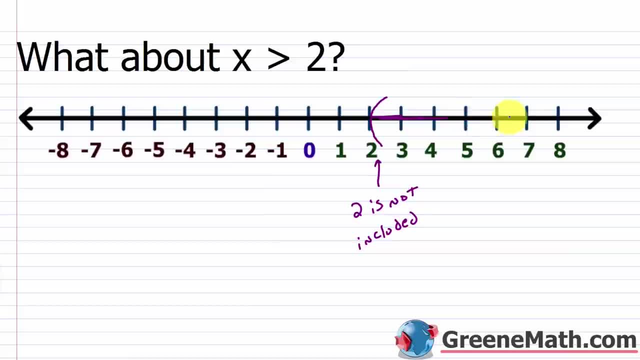 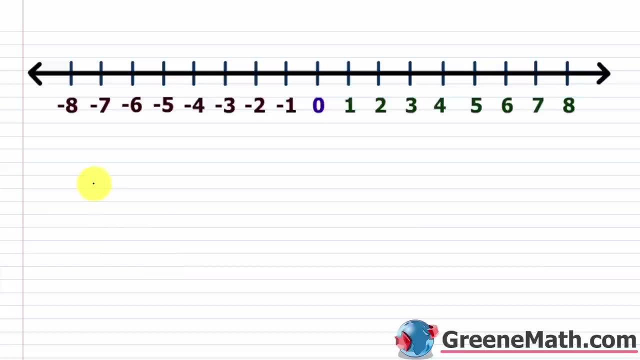 so I'm gonna shade all this and when you're doing this on a test, just make it clear that you're shading everything to the right and just shade that arrow there just to say, hey, this is gonna continue forever and ever and ever. let's try another one. let's say we had something like X is greater than 4, so X. 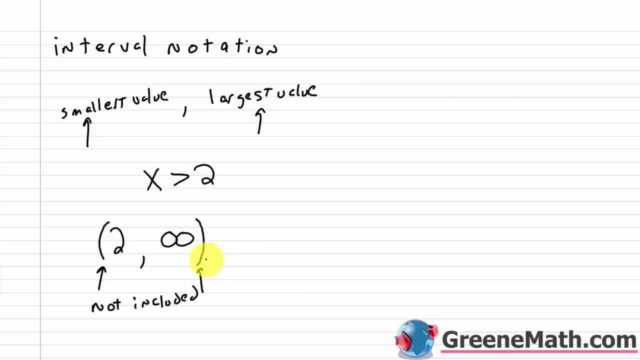 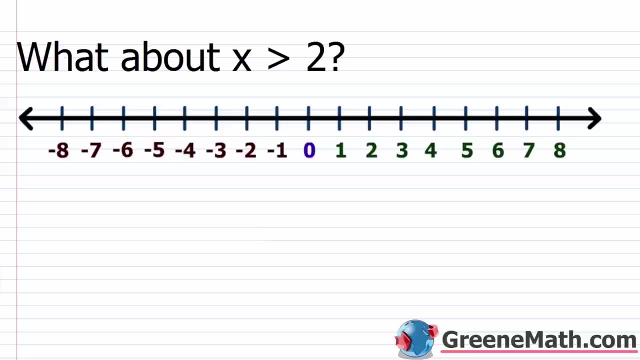 How do we use this to graph? Well, it's similar. If I have x is greater than 2, I find 2 on the number line. And what I'm going to do is I'm going to put a parenthesis at 2 that faces in the direction of my solution. So this is going to face to the right because everything larger than 2 is in the solution. 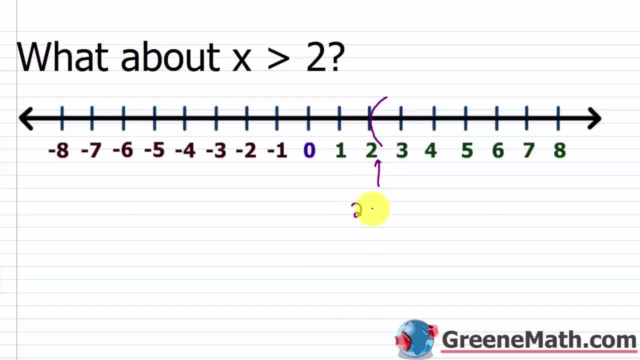 The parenthesis is telling me that 2 is not included. 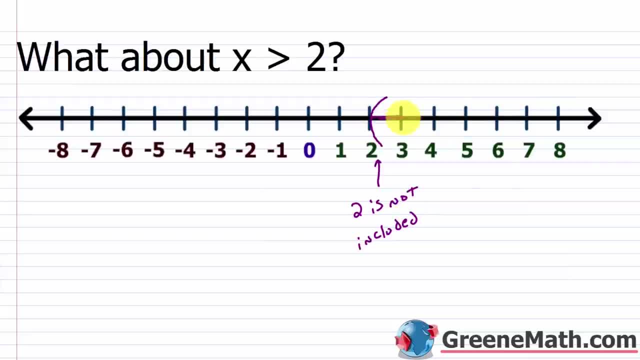 And then I'm going to shade everything to the right. So I'm going to shade all this. And when you're doing this on a test, just make it clear that you're shading everything to the right. Just shade that arrow there just to say, hey, this is going to continue forever and ever and ever. 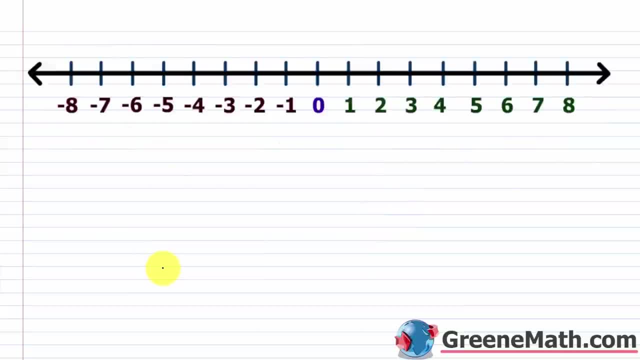 Let's try another one. Let's say we had something like x is greater than 4. So x is greater than 4. 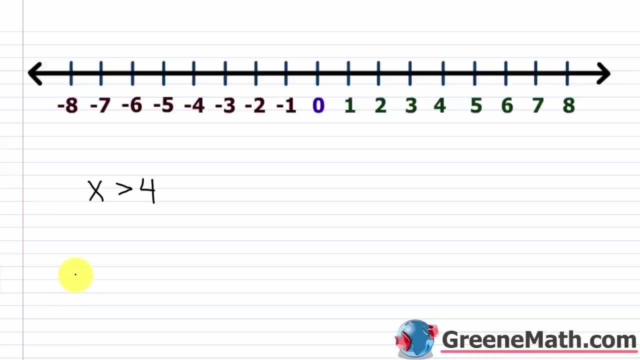 So in interval notation, again, you want the smallest value on the left. Now, I can't possibly list the actual smallest value because, again, I can't get to it. Anything that I could 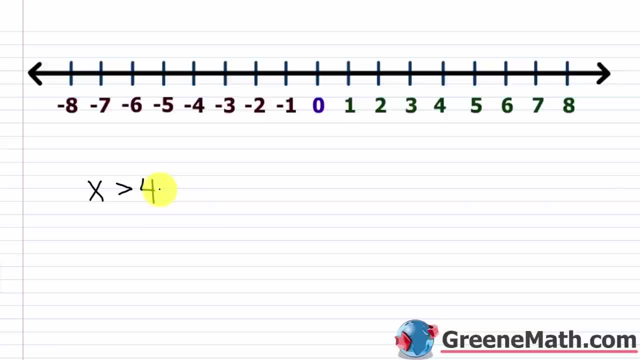 list that's the smallest value could always get smaller. So I'm just going to go ahead and put 4. 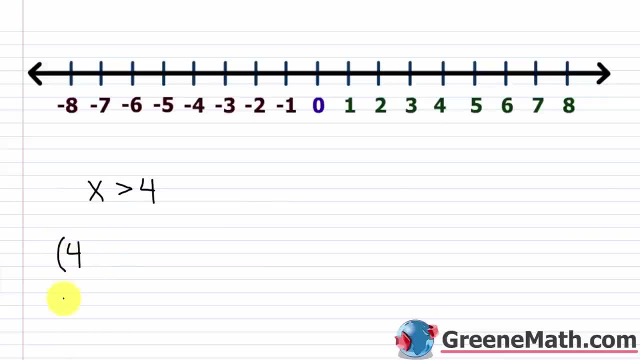 And I'm going to put a parenthesis next to 4 to say that it's not included. It's not included. 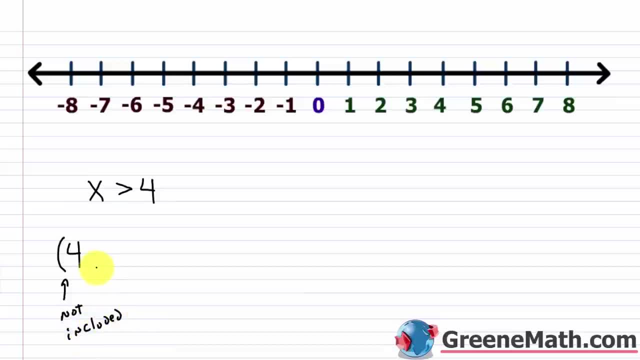 But hey, anything larger than that is. So then I put my comma, and then my largest value. 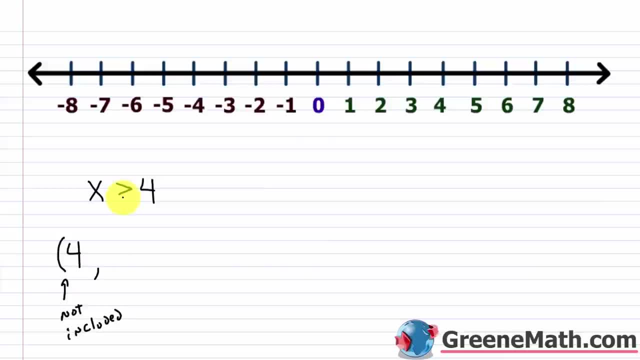 And again, because x can be anything larger than 4, there is no 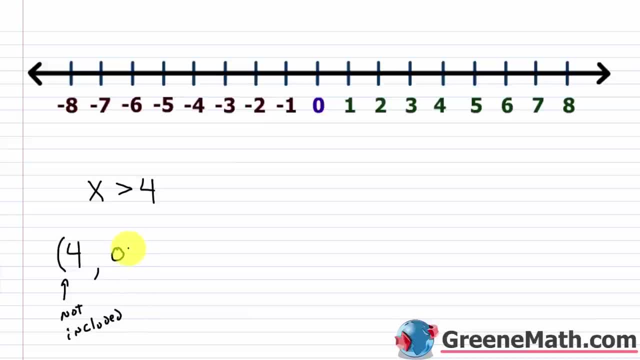 largest value. So we're going to put the infinity symbol in. Again, it looks like a sideways 8. 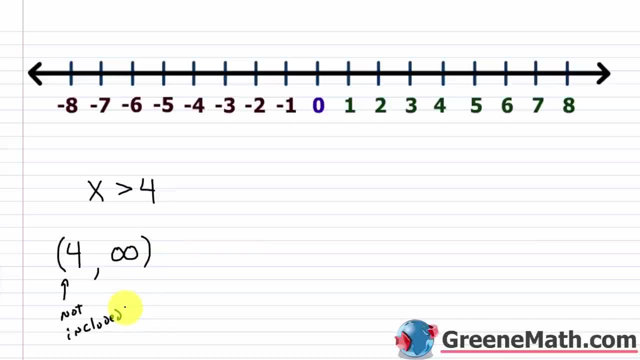 We put our infinity symbol in. And again, we put a parenthesis to say, hey, it's not included. And then graphically, we're looking for 4 on the number line. We're going to put a parenthesis there at 4 to say, hey, 4 is not included. That means not included. 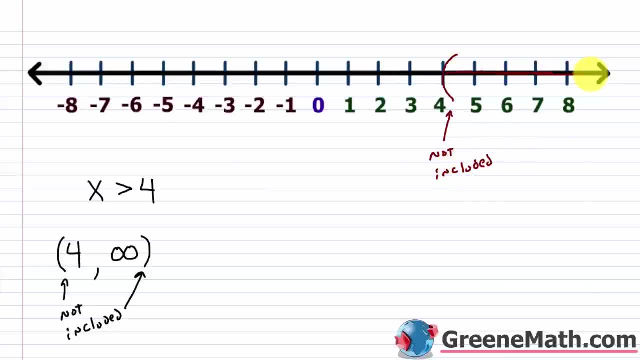 And then we're going to highlight all this. We're going to highlight that arrow to say, hey, this solution is going to continue forever and ever and ever in that right 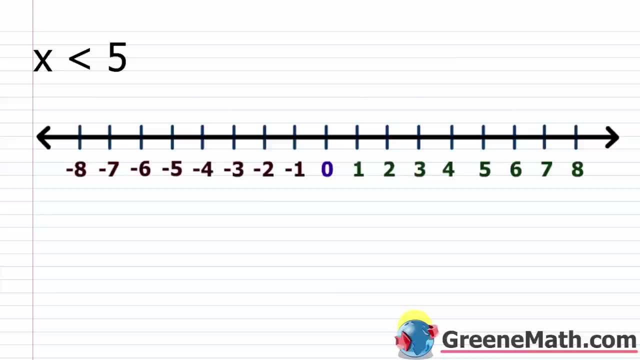 direction. So what about something like x is less than 5? 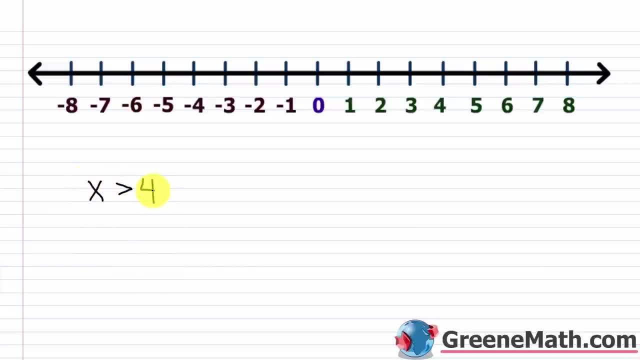 is greater than 4. so in interval notation again you want the smallest value on the left. now I can't possibly list the actual smallest value because, again, I can't get to it. I know anything that I could list. that's the smallest value. it could always get smaller, so I'm just gonna go ahead and put 4 and I'm 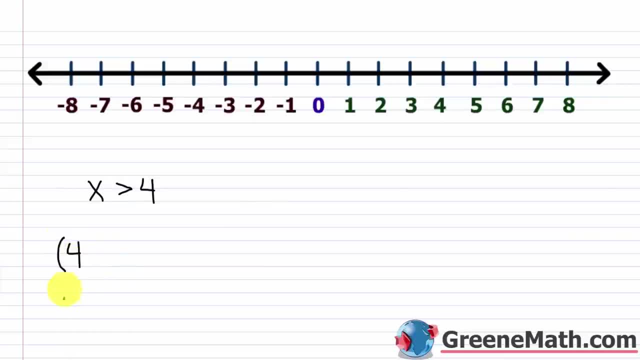 gonna put a parenthesis next to 4 to say that it's not included. it's not included, but hey, anything larger than that is. so then I put my comma and then my largest value and again, because X can be anything larger than 4, there is no. 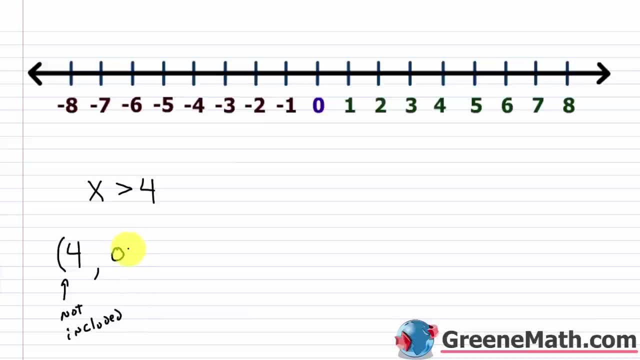 largest value. so we're gonna put the infinity set symbol in. again it looks like a sideways 8. we put our infinity symbol in and again we put a parenthesis to say hey, it's not included. and then graphically we're looking for 4. on the number line we're gonna put a. 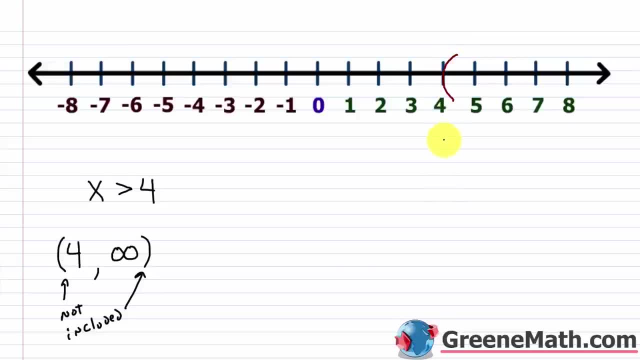 parenthesis there at 4 to say, hey, 4 is not included, that means not included. and then we're gonna highlight all this, we're gonna highlight that arrow to say, hey, this solution is gonna continue forever and ever and ever in that right direction. so what about something like: X is less than 5? well, if 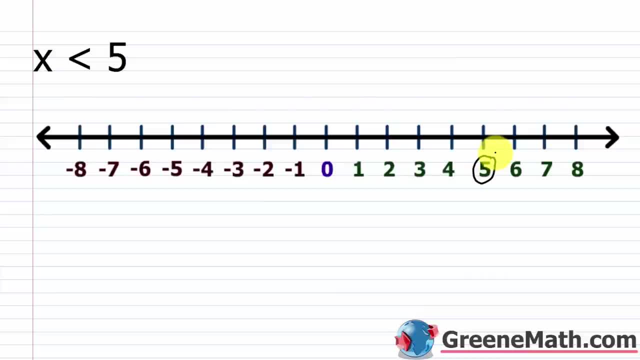 I look at my number line here, I see 5 is here. so X can be anything less than 5. it can't be 5 itself, but any value lower than that. so if I was to notate this, what is my smallest value? what is my smallest value? well, there's not gonna be. 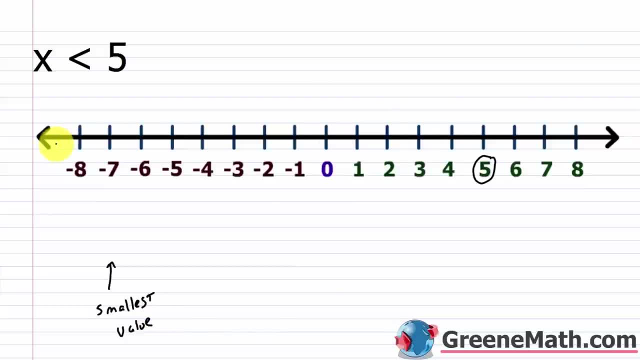 one right, because I can keep going to the left forever and ever and ever. so we're gonna notate this, using the concept that if I put the number line on it all the way here, it would stay the same right and, as you can see, as we 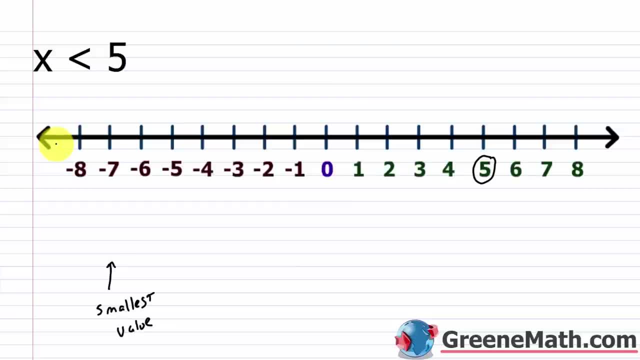 said, I immediately come up with the start sign in and what I'll do is I can menu all these formatted themes so we can get the same number line right. so the lineین'm going to have. so we're going to need tracta quem we'll 对. 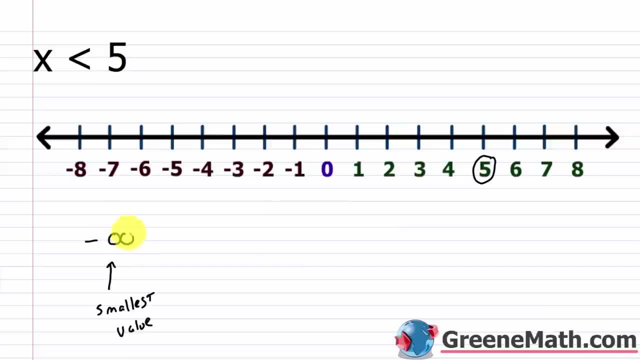 And then you put your infinity symbol. Remember, that's just a sideways-looking 8.. Now, because infinity is a concept. infinity or negative infinity, it's not really a number, It's a concept. You can't really include it. 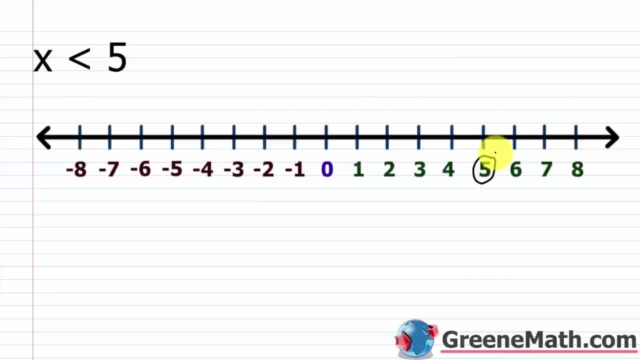 Well, if I look at my number line here, I see 5 is here. So x can be anything less than 5. It can't be 5 itself, but any value lower than that. So if I was to notate this, what is my smallest value? What is my smallest 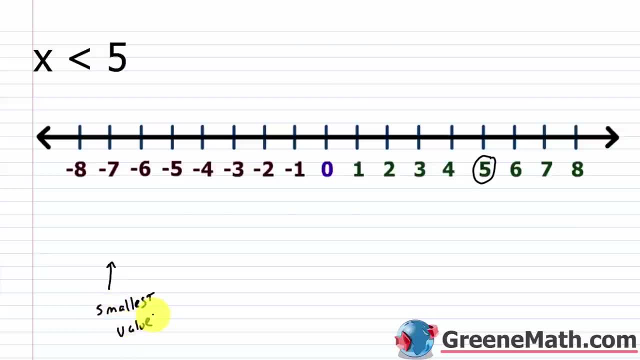 value? Well, there's not going to be one because I can keep going to the left forever and ever and ever. So we're going to notate this using the concept of negative infinity. Just like we had positive infinity to say, hey, numbers increase forever and ever and ever going to the right. So with positive infinity, whatever number I can think of, I can always add 1 to get to the next largest. 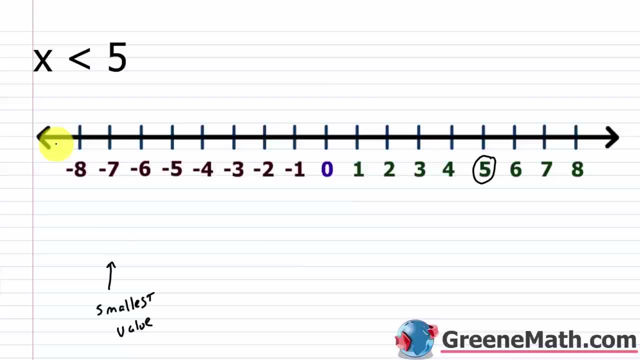 With negative infinity, whatever number I can think of, I can always subtract 1 and get to the next smallest. Numbers continue forever and ever in the left direction as well when we think about a number line. So a negative infinity looks like this. You put a negative and then you put your infinity symbol. 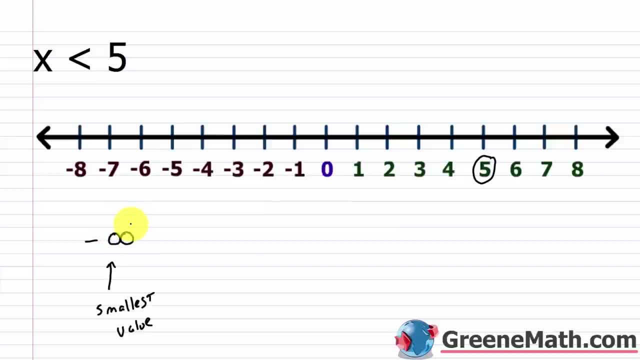 Remember, that's just a sideways looking 8. Now, because infinity is a concept, infinity or negative infinity, it's not really a number, it's a concept, you can't really include it. So you're always going to use a parenthesis next to them. 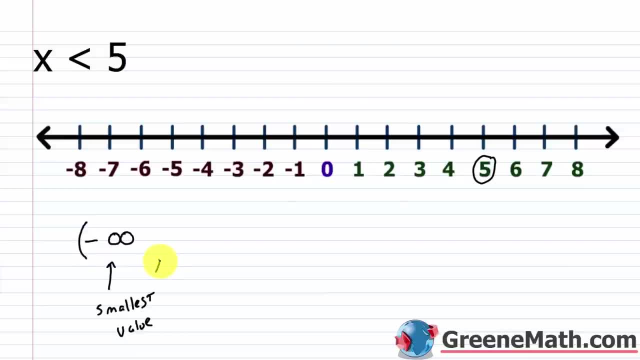 So I put a parenthesis there. Now, what's my largest value? What's my largest value? I know that x can be anything up to, but not including 5. 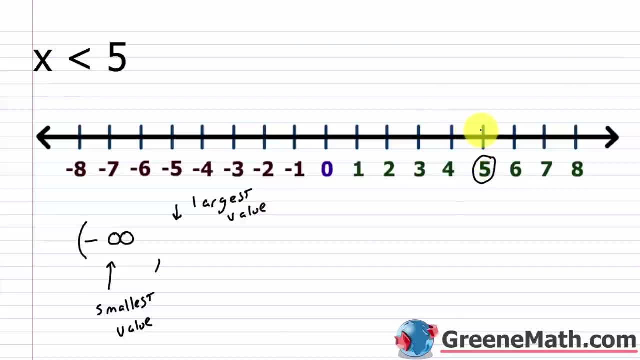 So if I look at the number line, I can get as close to 5 as I want, but I can never touch 5. So because I can't really list that as an actual number, I'm just going to use the number 5, and then I'm going to put a parenthesis next to it to again say that, hey, this is not included. This is not included. 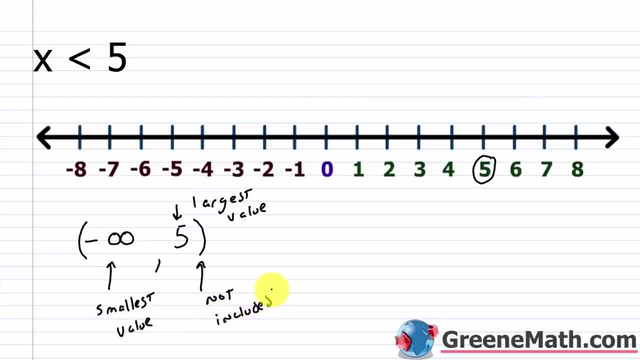 So anything smaller than 5 works, but I can't actually use 5. 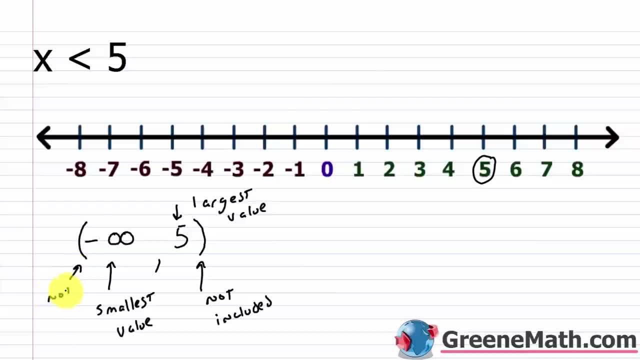 And let me put this over here too, that this is not included. 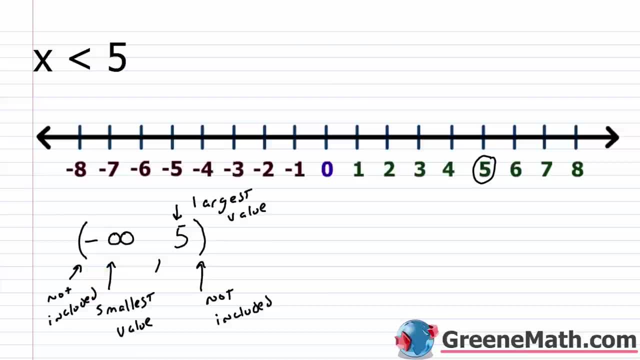 And then graphically, it's basically the same thing. 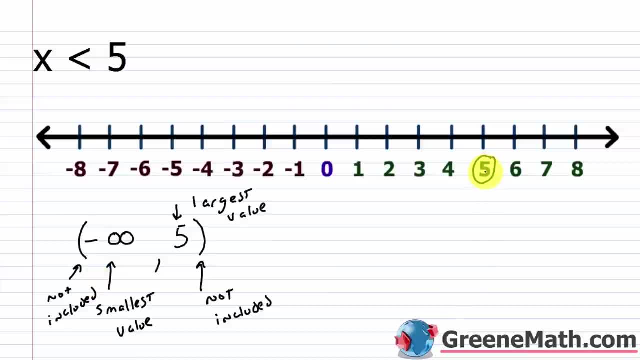 Now, I'm using a parenthesis at 5 to say that 5 is not included. 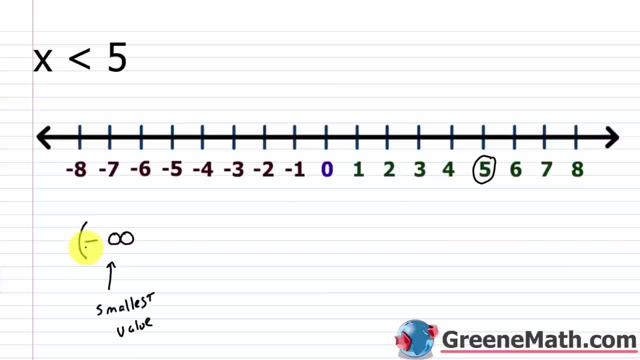 So you're always going to use a parenthesis next to them. So I put a parenthesis there. Now, what's my largest value? What's my largest value? I know that x can be anything up to, but not including 5.. So if I look at the number line, I can get as close to 5 as I want, but I can never touch 5.. 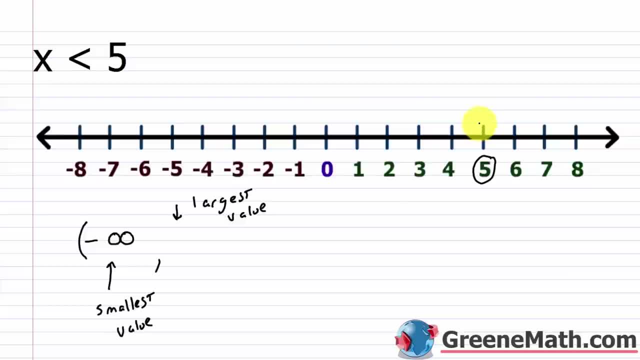 So, because I can't really list that as an actual number, I'm just going to use the number 5.. And then I'm going to put a parenthesis next to it to again say that hey, this is not included, This is not included. 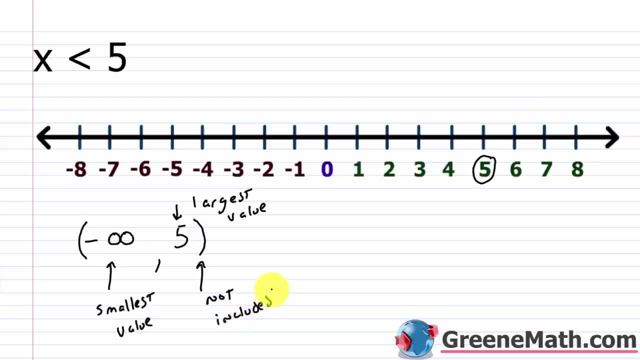 So anything smaller than 5 works, But I can't actually use 5.. And let me put this over here too, that this is not included. And then graphically it's basically the same thing. Now I'm using a parenthesis at 5 to say that 5 is not included. 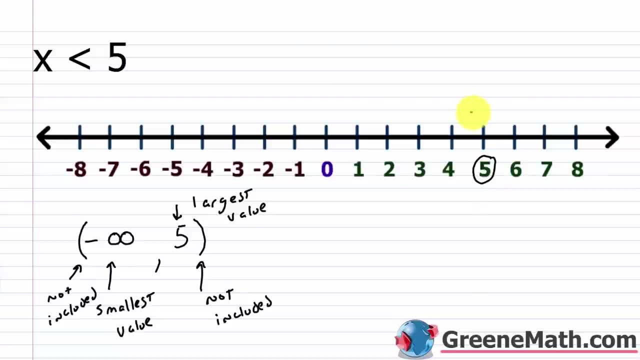 But notice how now I'm going to point the parenthesis towards the left, because my solution goes to the left. And now I'm just going to shade all of this And then make sure you shade that arrow And to say, hey, this is going to continue forever and ever and ever in the left direction. 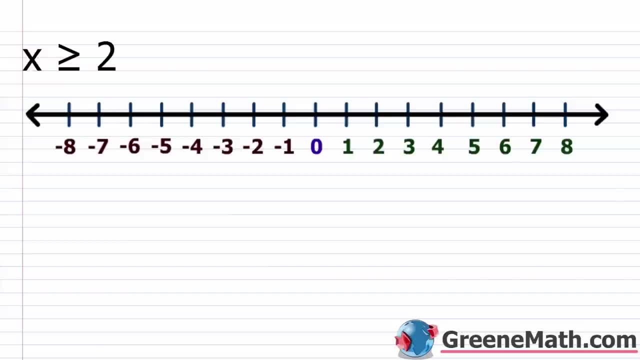 All right. So when we have a non-strict inequality, we're going to use a bracket next to the number that's included. So this is the biggest thing we need to remember. So now we're looking at. x is greater than or equal to 2.. 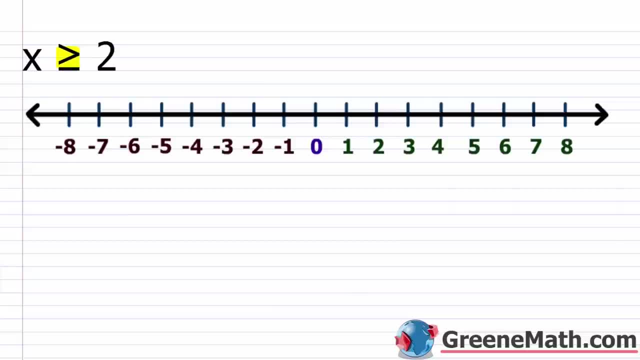 Or equal to 2.. Very important, you understand the difference. So when I look at my number, line x can be 2. now It can actually be equal to 2.. That can be a solution. It can also be anything larger than 2.. 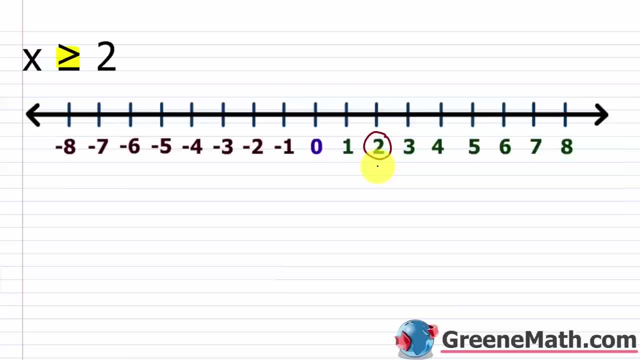 Just like with the strict inequality. So in this particular case, when we're writing out our solution and interval notation, the smallest possible value that x can take on is actually 2.. And I put a bracket there to say that 2 is included. 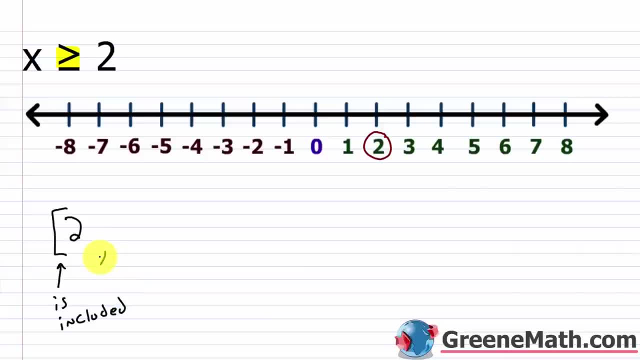 Now comma. Now, what's the largest value that x can take? Well, again, it's going to be infinity, right? Just because I have a non-strict inequality doesn't mean that both of them are going to have a bracket. x is anything that is greater than or equal to 2.. 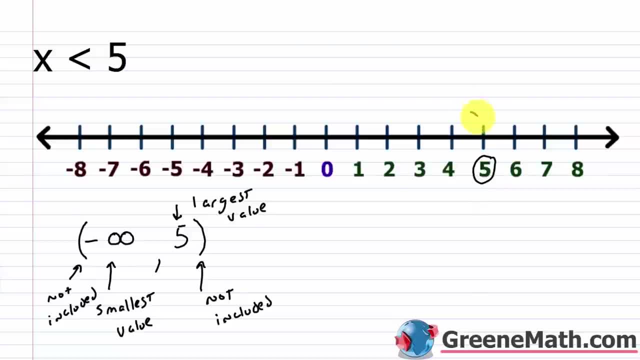 But notice how now I'm going to point the parenthesis towards the left, because my solution goes to the left. And now I'm just going to shade all of this and then make sure you shade that arrow in to say, hey, this is going to continue forever and ever and ever in the left direction. 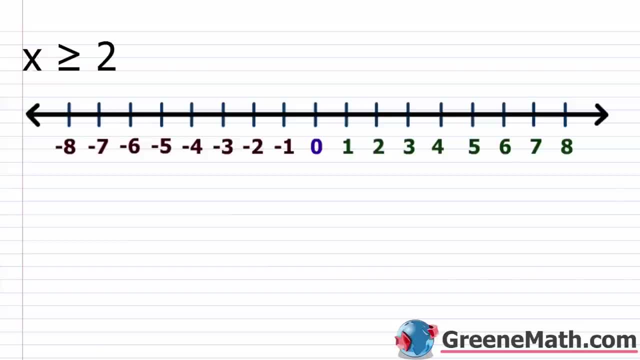 Alright, so when we have a non-strict inequality, we're going to use a bracket next to the number that's included. 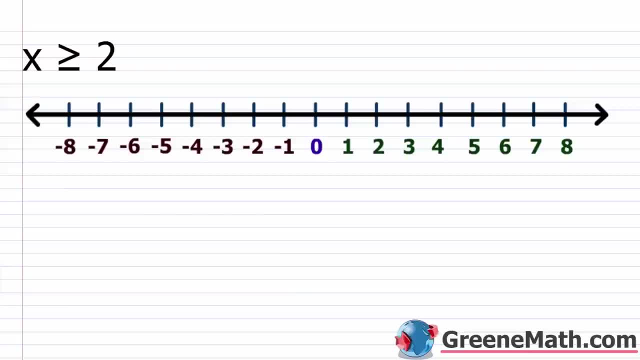 So this is the biggest thing we need to remember. So now we're looking at x is greater than or equal to 2. Or equal to 2. Very important you understand the difference. 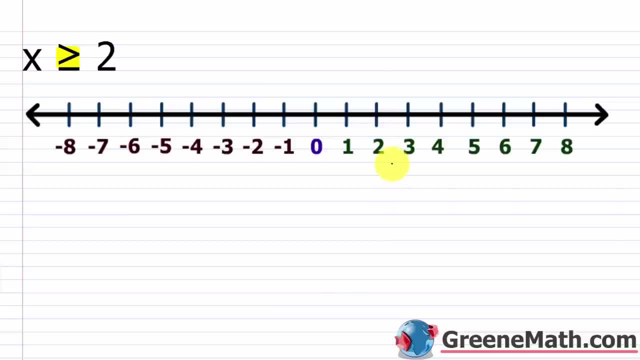 So when I look at my number line, x can't be 2 now. It can actually be equal to 2. That can be a solution. It can also be anything larger than 2. Just like with the strict inequality. So in this particular case, when we're writing out our solution and interval notation, the smallest possible value that x can take on is actually 2. 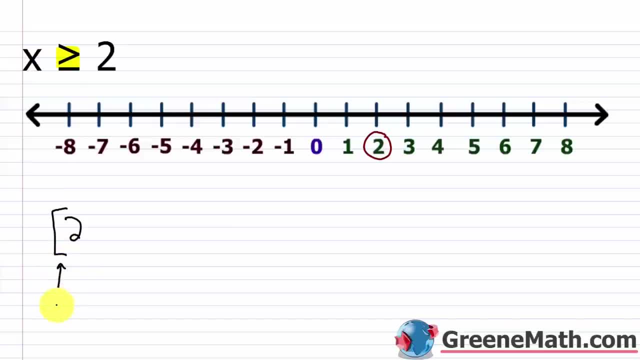 And I put a bracket there to say that 2 is included. 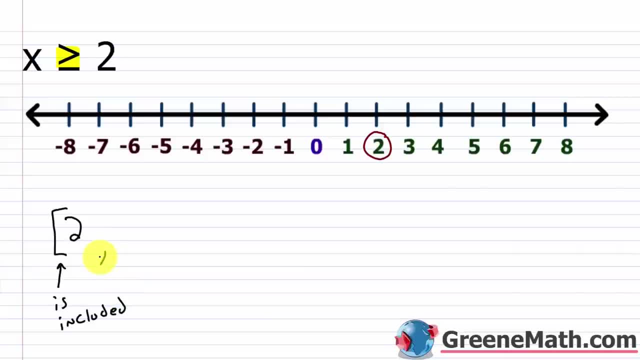 Now comma Now what's the largest value that x can take on? 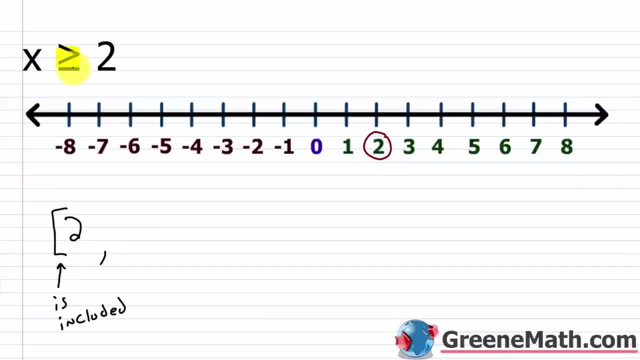 Well again, it's going to be infinity. Just because I have a non-strict inequality doesn't mean that both of them are going to have a bracket. 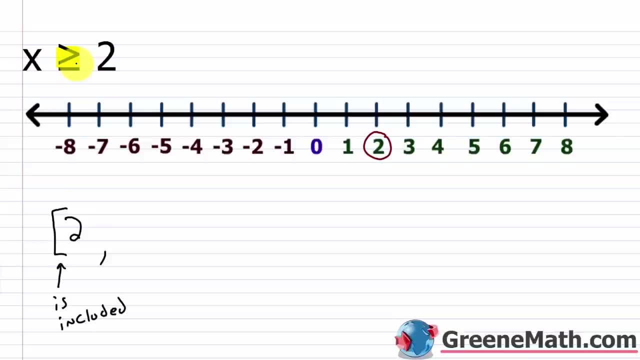 x is anything that is greater than or equal to 2. So x still goes out forever and ever and ever in the right direction. So we're going to use infinity here to notate that and then you always put a parenthesis there and again this is not included. Okay? 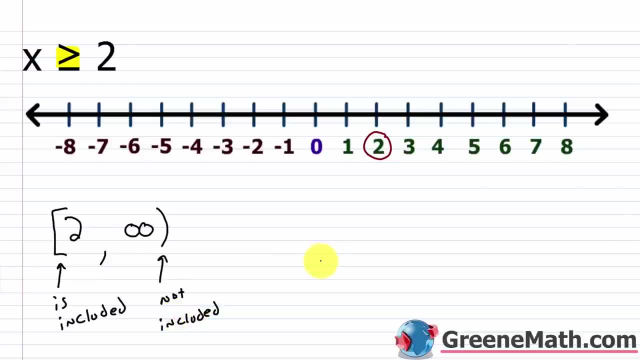 So now graphically you're going to change things up a little bit. 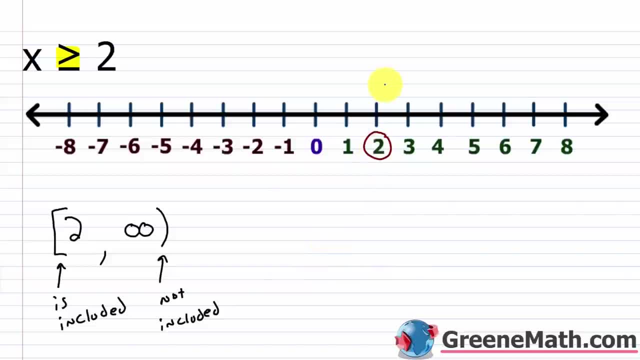 So at 2 instead of a parenthesis you're putting a bracket. And that bracket faces in the direction of the solution. That's going to face this way and then I'm going to shade everything to the right including that arrow to say hey 2 is included is included and then also anything to the right of 2. 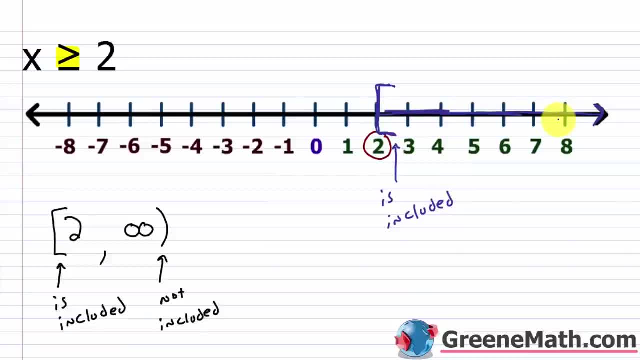 So 2 itself and then anything to the right of 2 continuing out forever and ever and ever out to infinity. 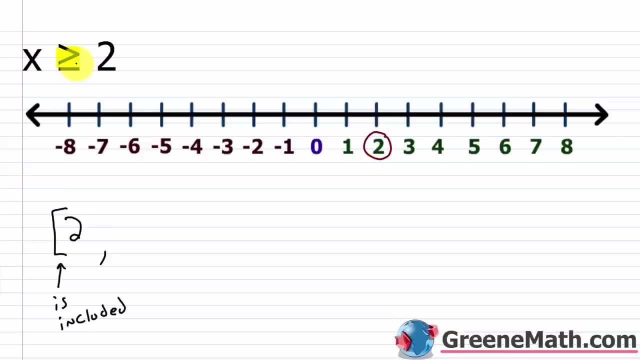 So x still goes out forever and ever and ever in the right direction. So we're going to use infinity here to notate that. And then you always put a parenthesis there And again, this is not included. Okay, So now graphically. 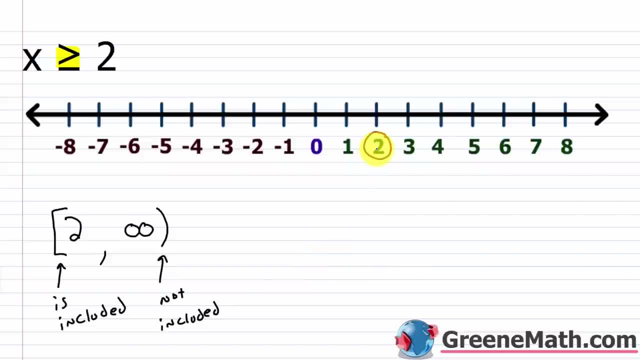 you're going to change things up a little bit. So at 2,, instead of a parenthesis, you're putting a bracket, And that bracket faces in the direction of the solution That's going to face this way, And then I'm going to shade everything to the right. 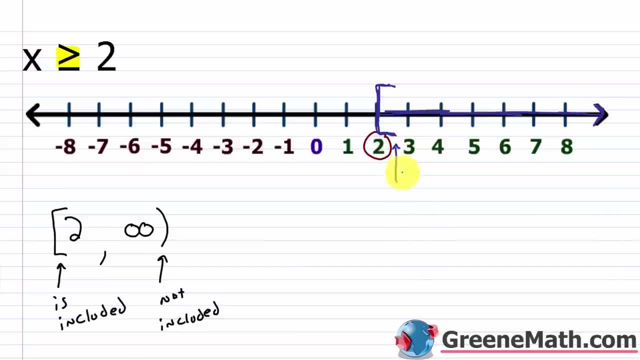 including that arrow to say, hey, 2 is included, Is included, And then also anything to the right of 2.. Okay, so, 2 itself, and then anything to the right of 2, continuing out Forever and ever, and ever, out to infinity. 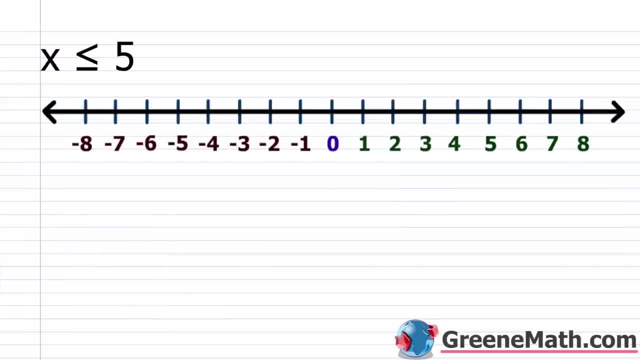 What about x is less than or equal to 5?? So again, here's 5 on the number line. So now x can be 5 or anything less than 5.. So when we think about writing our solution in interval notation, the smallest possible value is still the same. 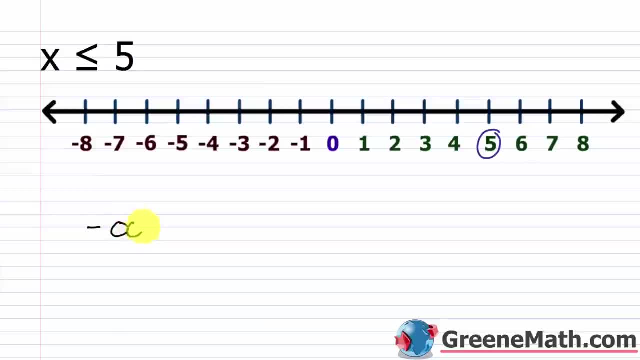 The smallest possible value is still negative infinity. Right, because we can have x as anything, that's 5 or less And that continues to the left, forever and ever and ever. So we still have negative infinity and we still use a parenthesis next to that. 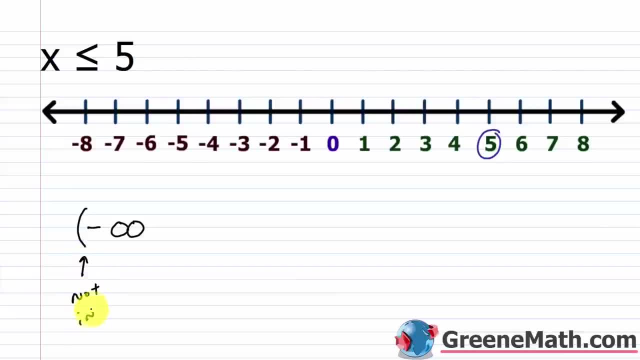 to say, hey, this is not included. Then we have comma. Now what's the largest value that x can take on? Well, x can take on the value of 5 now, but nothing larger. So I'm going to put the number 5,. 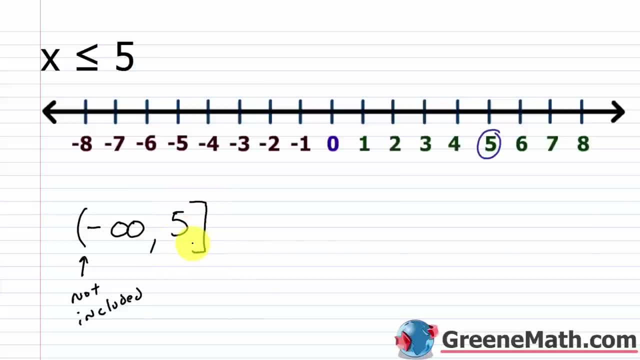 and I'm going to put a bracket next to 5 to say that 5 is included. So, basically, what you need to take away from this is that a bracket tells you it's included, parenthesis tells you it's not included, And to graph this again, very, very simple: 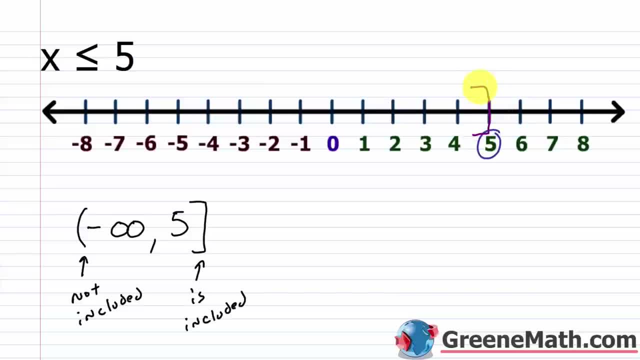 You put a bracket at 5, and it's going to face in the direction of the solution region, So 5 is included. That's why we use the bracket. We just shade everything to the left, Everything to the left, Shade the arrow. 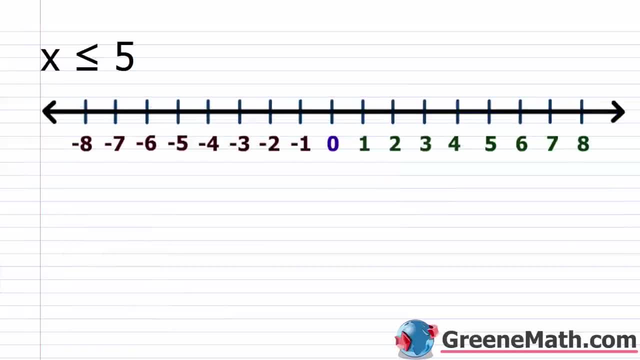 What about x is less than or equal to 5? So again here's 5 on the number line. So now x can be 5 or anything less than 5. 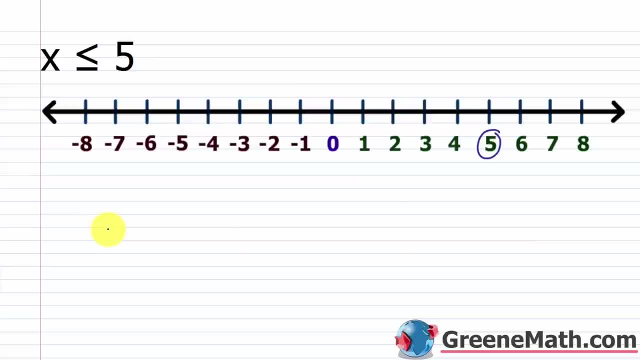 So when we think about writing our solution in interval notation the smallest possible value is still the same. The smallest possible value is still negative infinity. 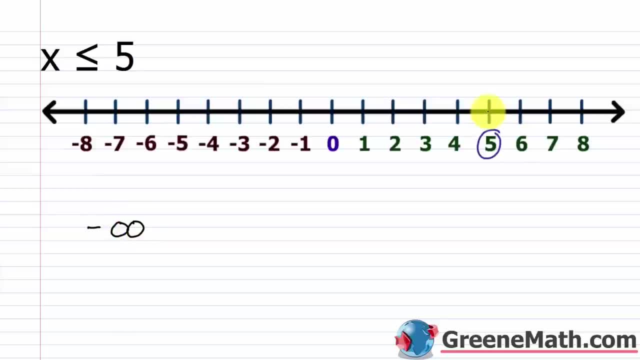 Because we can have x as anything that's 5 or less. And that continues to the left forever and ever and ever. So we still have negative infinity and we still use a parenthesis next to that to say hey this is not included. 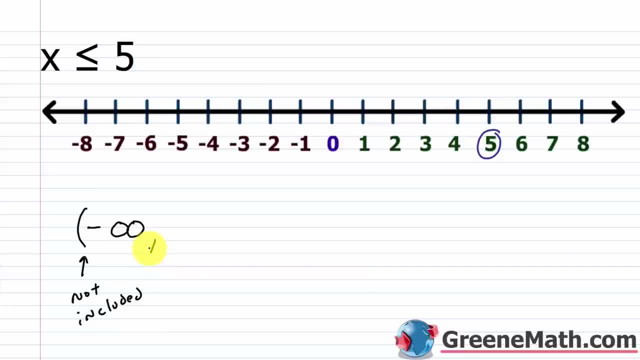 Then we have comma now what's the largest value that x can take on? Well x can take on the value of 5 now but nothing larger. So I'm going to put the number 5 and I'm going to put a bracket next to 5 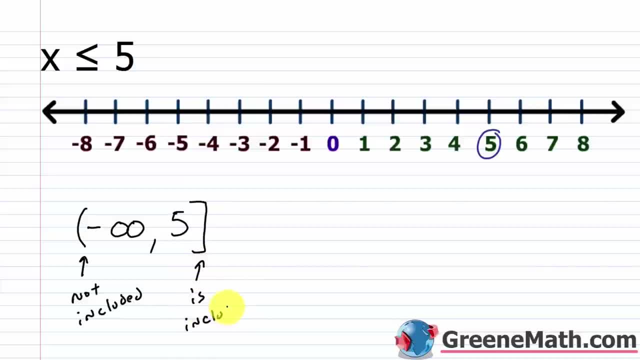 to say that 5 is included. So basically what you need to 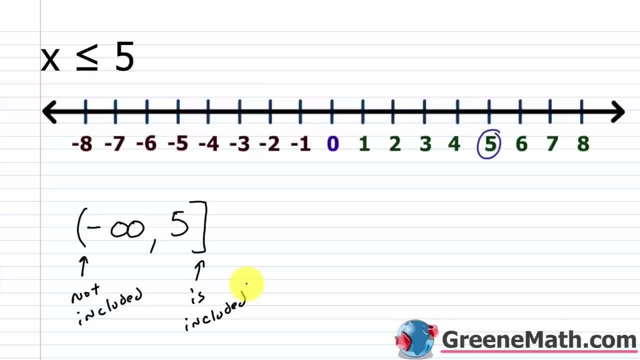 take away from this is that a bracket tells you it's included parenthesis tells you it's not included. 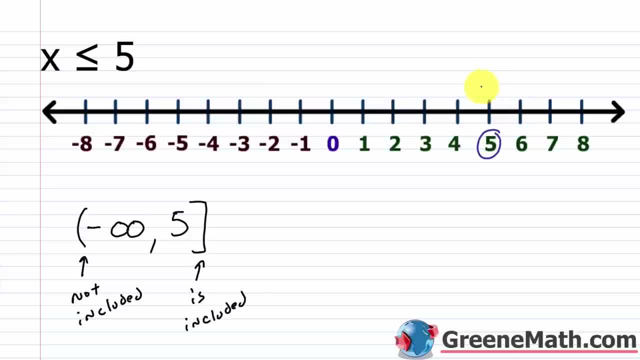 And to graph this again very very simple you put a bracket at 5 and it's going to face in the direction of the solution region. 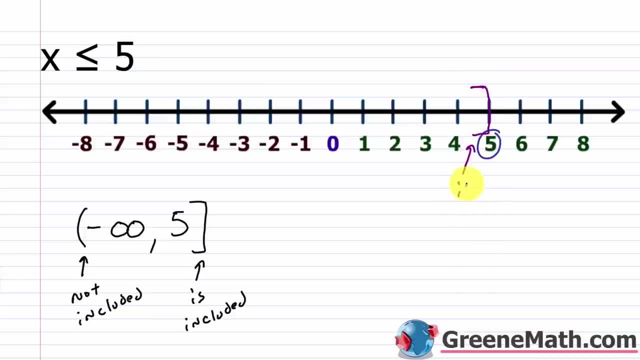 So 5 is included that's why we use the bracket 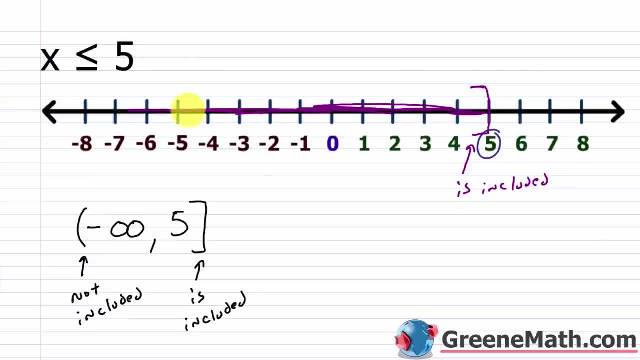 and we just shade everything to the left. Everything to the left. 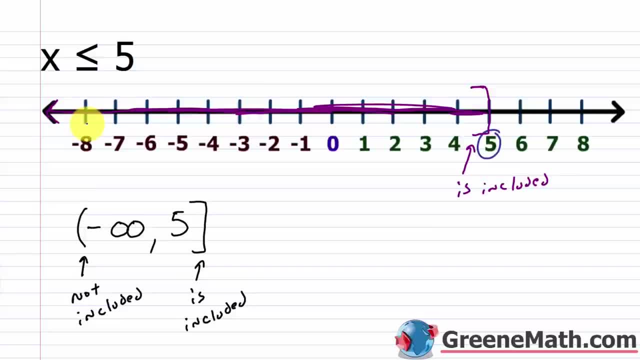 Shade the arrow because this continues forever and ever and ever in that direction. 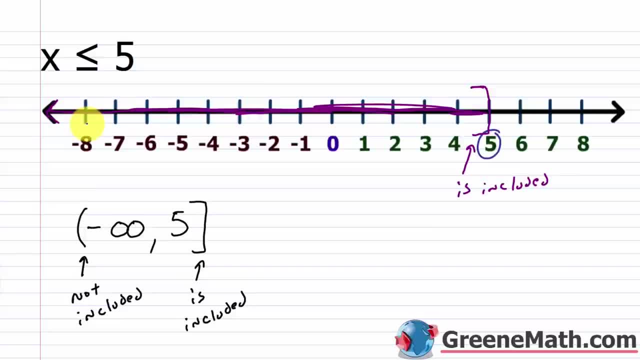 So again the main take away here is that if you're using a parenthesis you're saying that the number is not included. 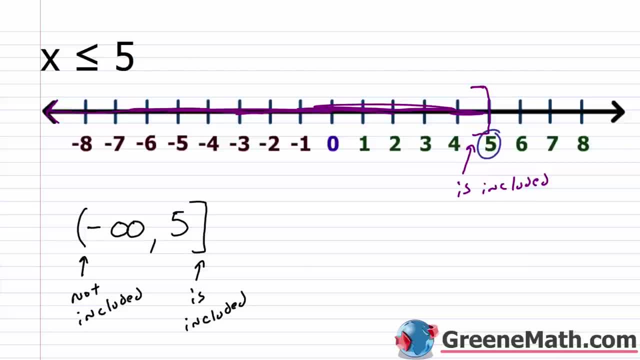 If you're using a bracket you're saying it is included. Now not to confuse you but I want to cover something that your teacher 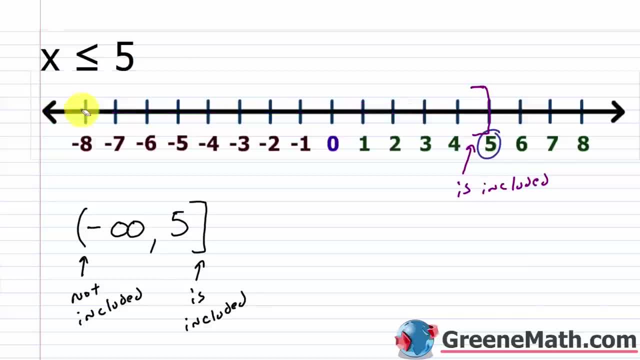 or your textbook might do. So I want to erase this real quick just the graphing part. Your teacher, your textbook, your tutor whoever you're using to learn this information may do things a little bit differently. 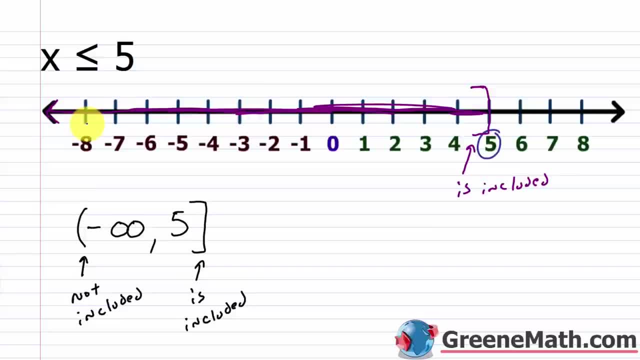 Because this continues forever and ever and ever in that direction. So again, the main takeaway here is that if you're using a parenthesis, you're saying that the number is not included. If you're using a bracket, you're saying it is included. 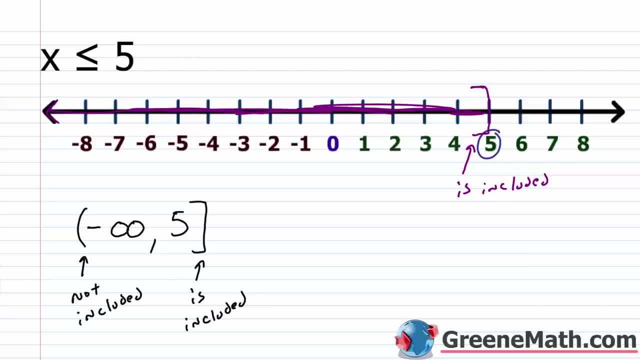 Now, not to confuse you, but I want to cover something that your teacher or your textbook might do, So I want to erase this real quick. Just the graphing part. Your teacher, your textbook, your tutor, whoever you're using to learn this information- 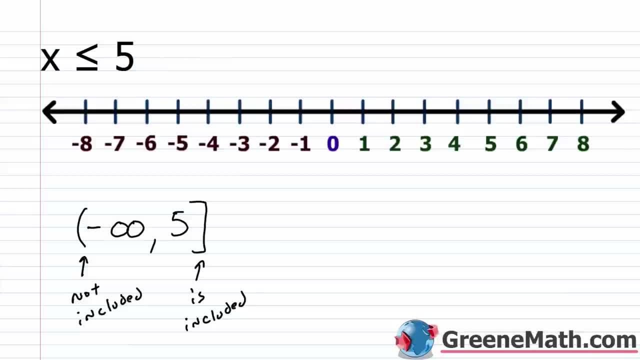 may do things like this. They may do things a little bit differently. When you graph things, you can do it in the way that I showed you: perfectly legal, perfectly acceptable, Or there's another way, Instead of using a bracket. 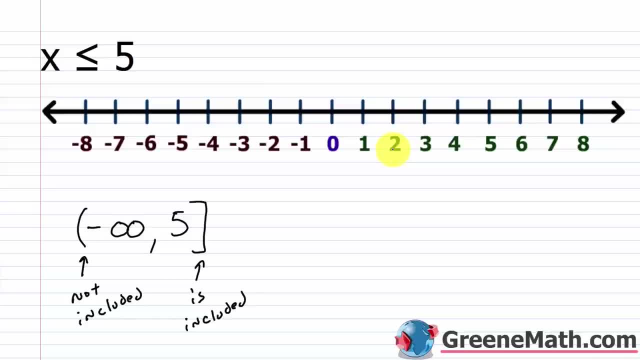 when something's included, you use a filled-in circle or a filled-in dot, So this means is included. If something's not included, you can use an open circle or an open dot, Meaning it's empty, It's not filled in. 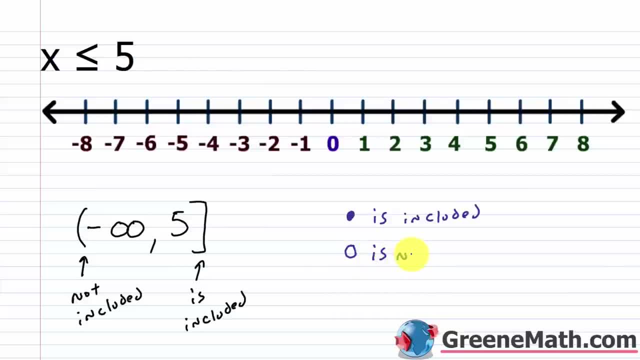 So this is not included. So, for example, if x is less than or equal to 5, I could show that graphically by kind of making a filled-in circle here and just going all the way to the left and highlighting this. This is the same as putting a bracket facing to the left. 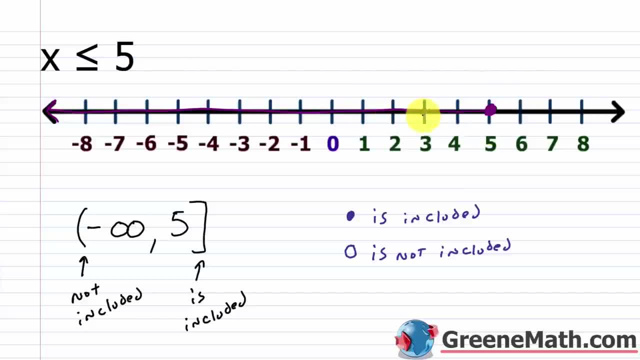 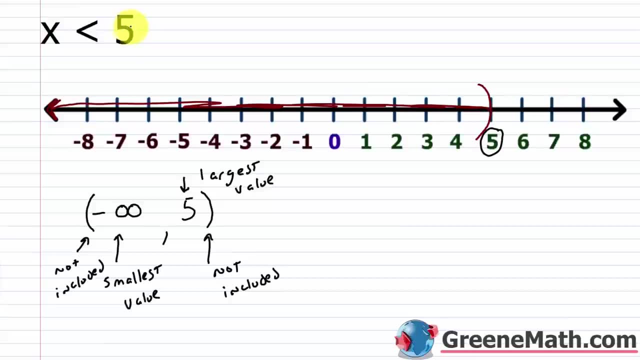 and shading to the left. You may see this in your textbook. As another example, we go back and revisit: x is less than 5.. And so again, instead of this parenthesis here, to say 5 is not included, what your teacher may do. 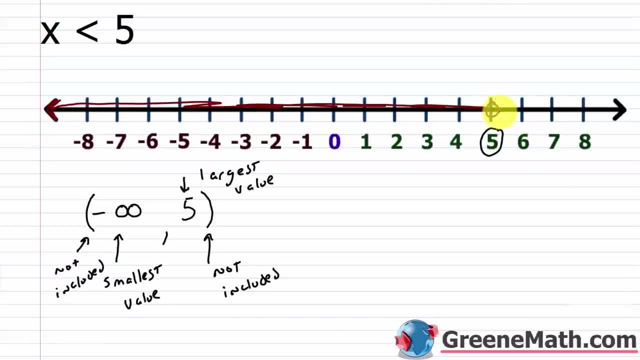 is put a circle at 5 that's not filled in. You see how there's a gap there. Let me make it a little bigger. Let me make it a little bit bigger. So let me just make that huge, And so you can see there's open. 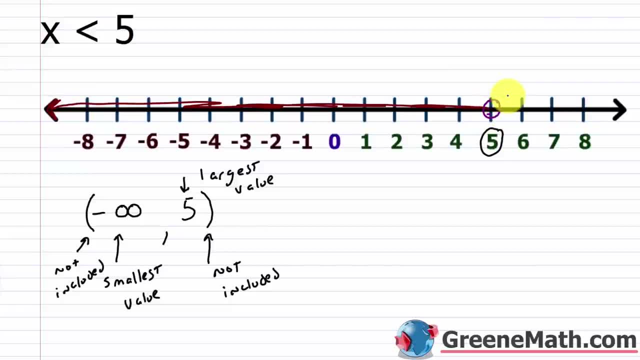 or a non-filled-in area there And your teacher may show you that. So this means 5 is not included. If I filled it in, it means 5 is included. So I just want to bring that to your attention, in case you're reading a book. 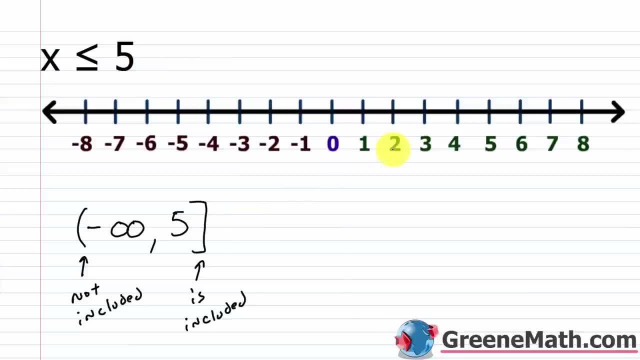 When you graph things you can do it in the way that I showed you perfectly legal, perfectly acceptable or there's another way. Instead of using a bracket when something's included you use a filled in circle or a filled in dot. So this means is included. 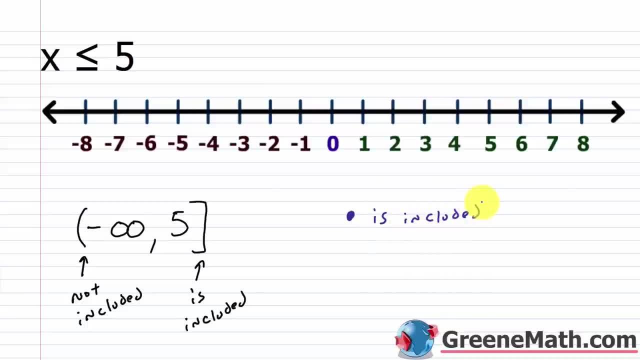 If something's not included you can use an open circle or an open dot meaning it's empty, it's not filled in. So this is not included. 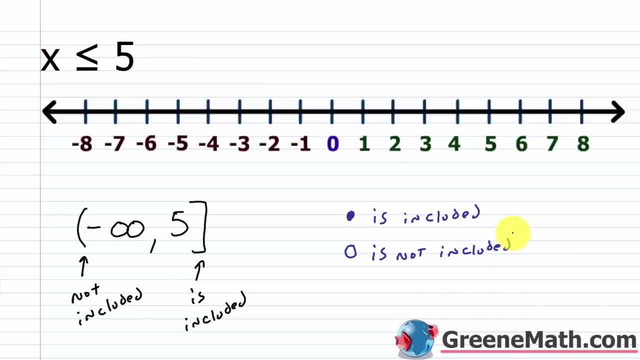 So for example if x is less than or equal to 5 I could show that graphically by kind of making a filled in circle here and just going all the way to the left and highlighting this. 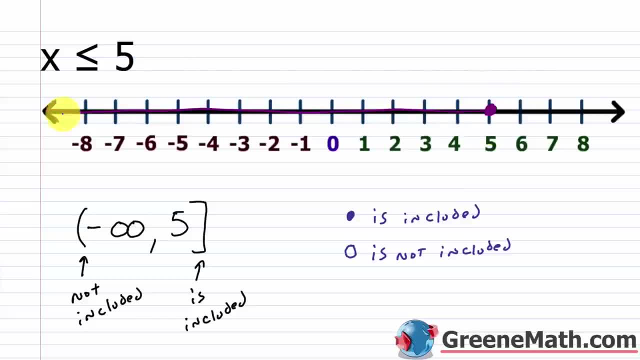 This is the same as putting a bracket facing to the left and shading to the left. You may see this in your textbook. 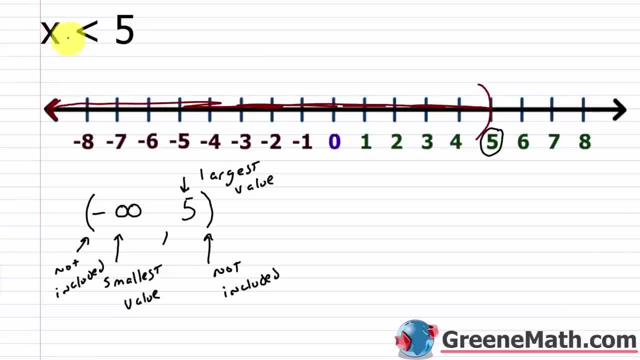 As another example we go back and revisit x is less than 5. And so again instead of this parenthesis 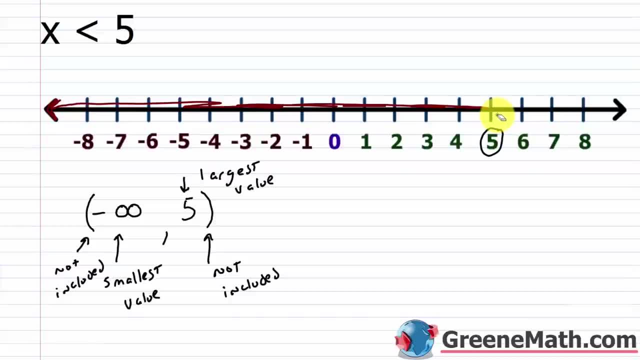 here to say 5 is not included what your teacher may do is put a circle at 5 that's not filled in. You see how there's a gap there? Let me make it a little bigger. 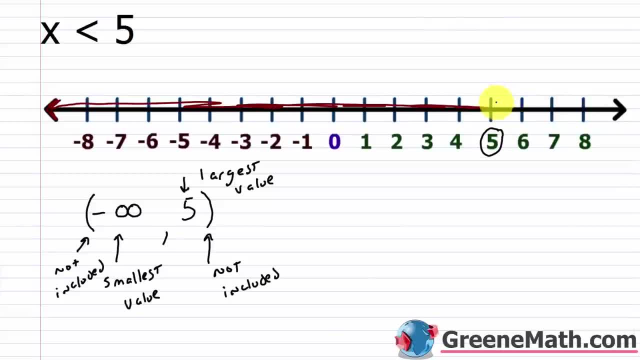 Let me make it a little bit bigger. So let me just make that huge. 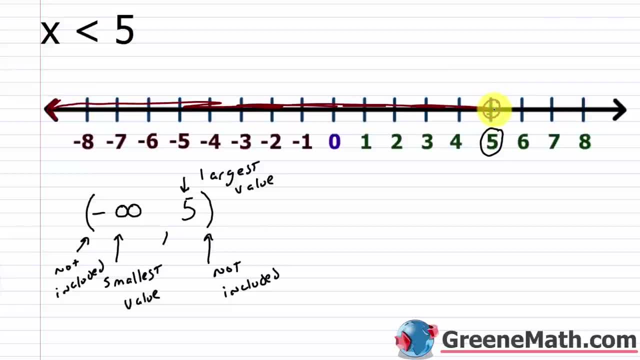 And so you can see there's open or non-filled in area there and your teacher may show you that. 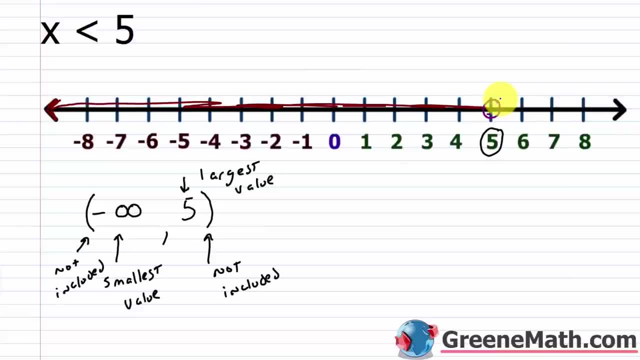 So this means 5 is not included. If I filled it in it means 5 is included. So I just want to bring that to your attention in case you're reading a book and it shows you a different way and you're like 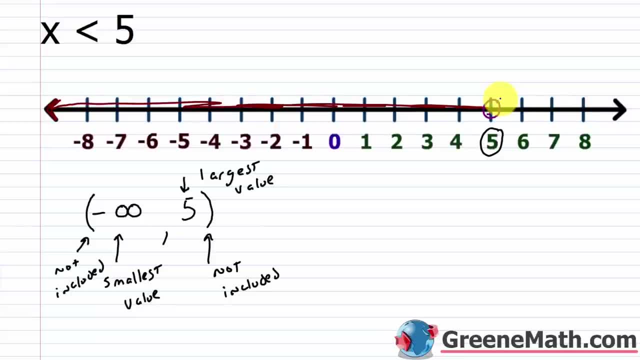 where'd that come from? Why is he doing it this way? Both ways are accepted and probably as you move higher the way that I'm showing you 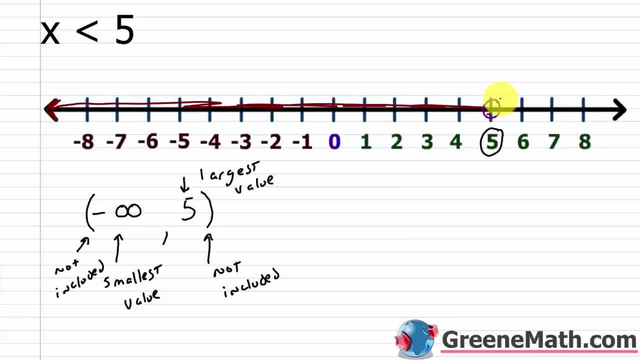 now is more accepted or used more often. I wouldn't say more accepted but used more often. 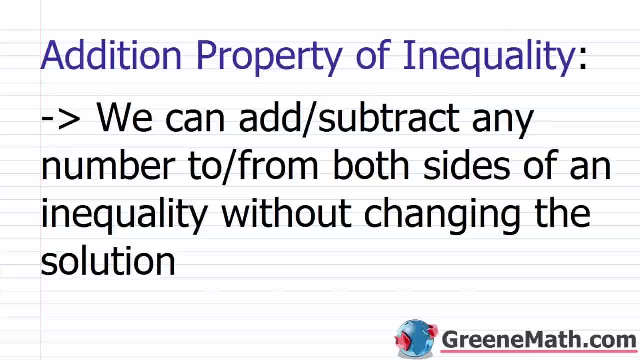 So now that we've gotten the basics out of the way let's cover a few things that you're going to need to know to be successful with solving a linear inequality in one variable. So the first thing is called the addition property of inequality. 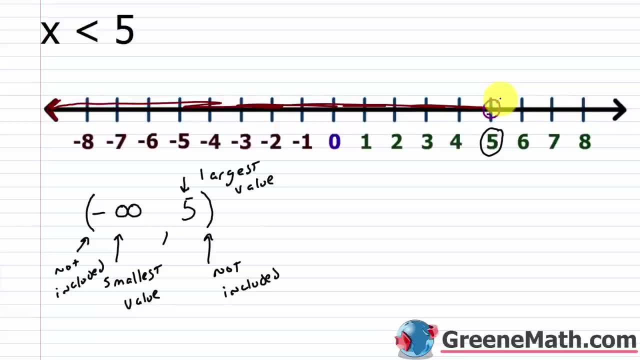 and it shows you a different way and you're like: where'd that come from? Why is he doing it this way? Both ways are accepted and probably, as you move higher, the way that I'm showing you now is more accepted or used more often. 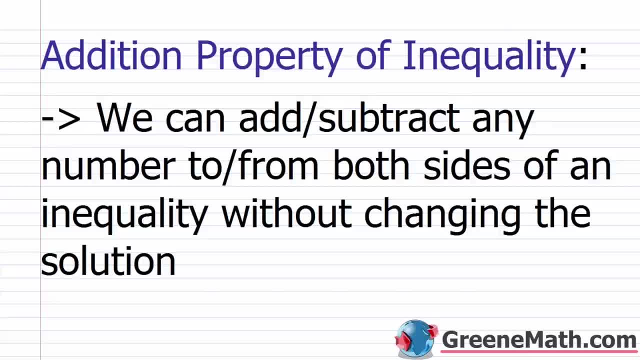 I wouldn't say more accepted, but used more often. So now that we've gotten the basics out of the way, let's cover a few things that you're going to need to know when solving a linear inequality in one variable. So the first thing is called the 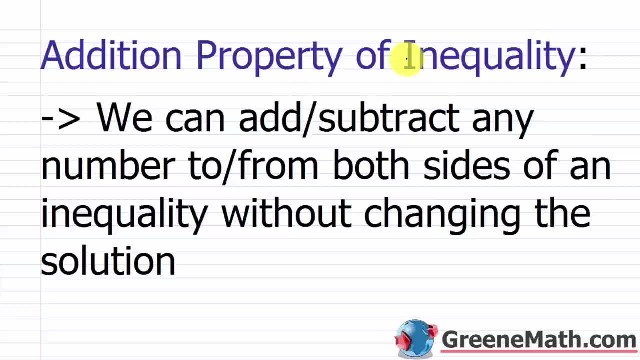 addition property of inequality, And you'll recall that we had an addition property of equality. Well, this is just for inequalities now. So it tells us we can add or subtract any number to or, in the case of subtraction, from both sides of an inequality, without changing the solution. 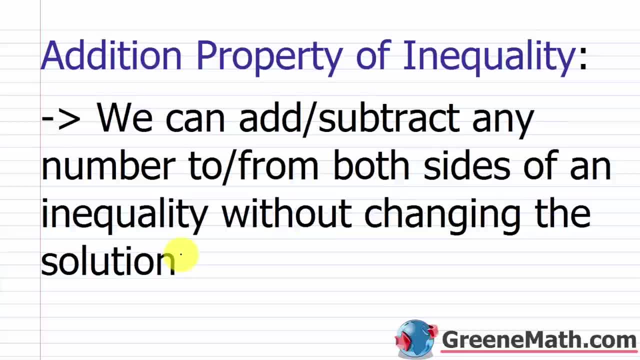 So that property that we use to solve equations where we added or subtracted the same number to or from both sides of the equation, can be extended to inequality. So we can now add or subtract the same number to or from both sides of an inequality. 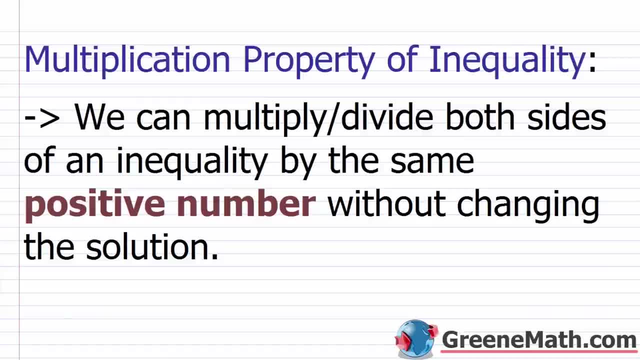 Now here's the other one, And this one is something you need to really pay attention to. We have the multiplication property of inequality, So I'm going to give you two different scenarios here. We can multiply or divide both sides of an inequality by the same positive number. 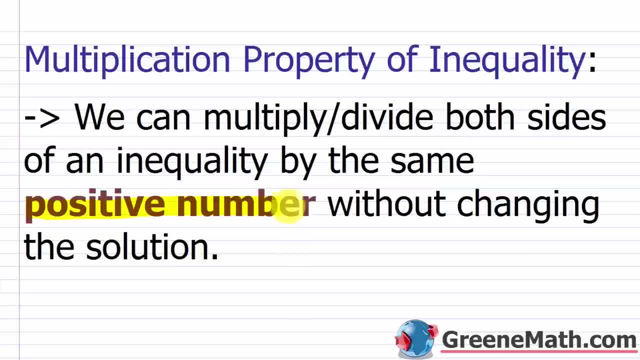 There's a reason. I put this in red and bold. So positive number, without changing the solution. So, just like the multiplication property of equality, the stipulation there was same non-zero number, You could multiply both sides of an equation by the same non-zero number. 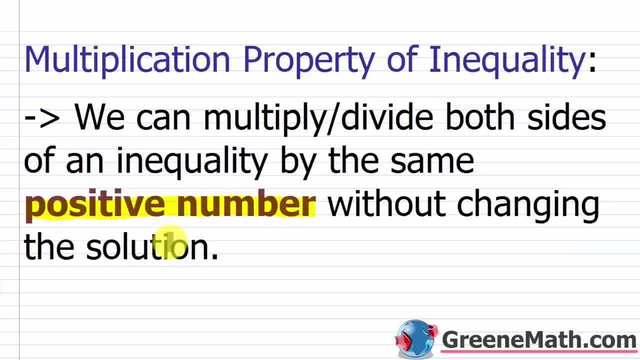 and you didn't change the solution Here. what I'm telling you is that you can multiply or divide both sides of an inequality by the same positive number, and positive does not include zero, for those of you who are thinking that It's positive or negative. 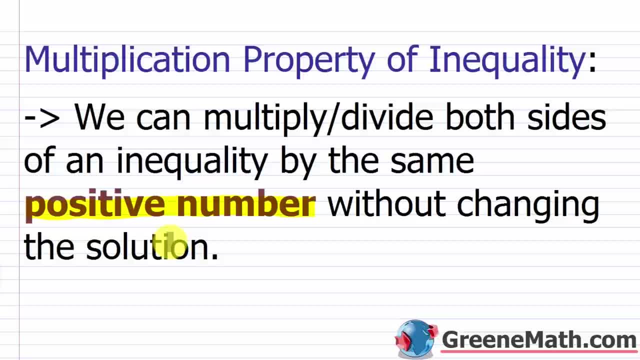 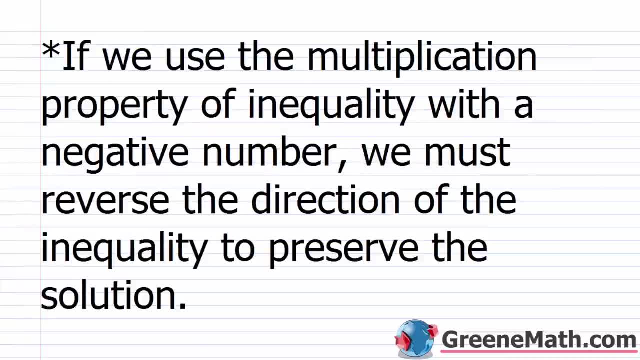 It's neither So by the same positive number without changing the solution. Here's where we run into problems, And I can't tell you how many tests I've graded in my life and I've seen students just not get this If we use the multiplication property. 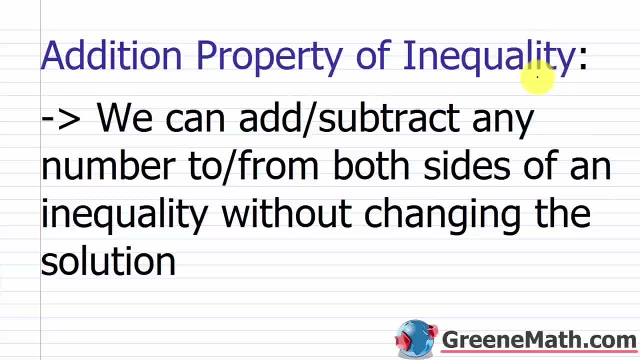 And you'll recall that we had an addition property of equality. Well this is just for inequalities now. So it tells us we can add or subtract any number to or in the case of subtraction from both sides of an inequality without changing the solution. So that property that we use to solve equations where we added or subtracted the same number to or from both sides of the equation can be extended to inequality. 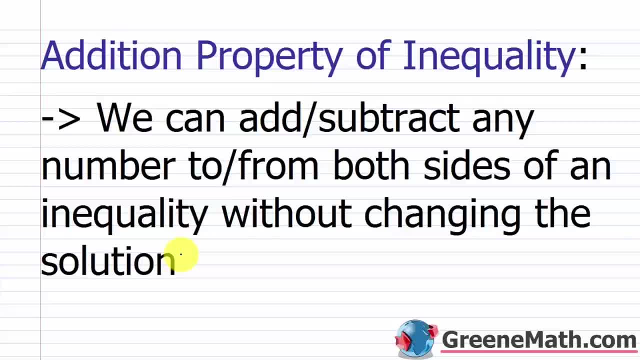 So we can now add or subtract the same number to or from both sides of an inequality. 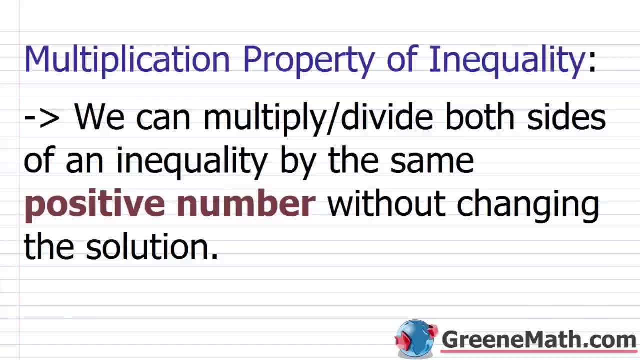 Now here's the other one and this one is something you need to really pay attention to. We have the multiplication 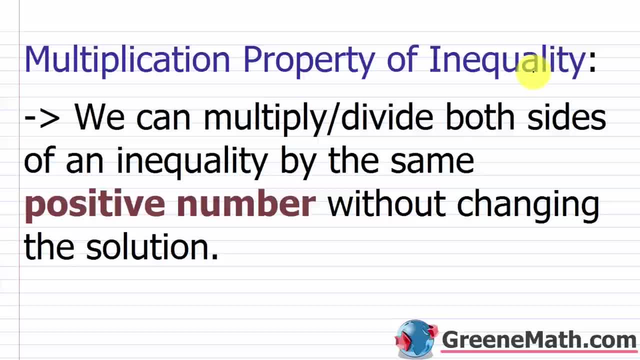 property of inequality. So I'm going to give you two different scenarios here. We can multiply or divide both sides of an inequality by the same positive number 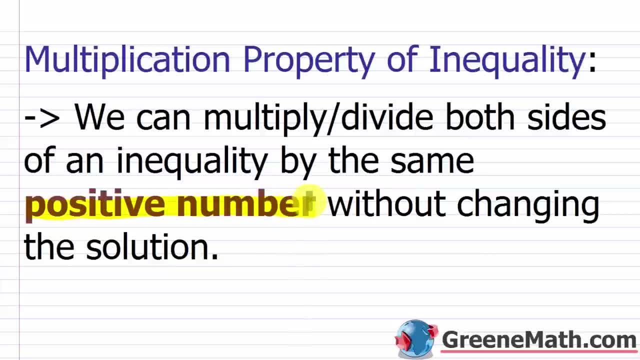 There's a reason I put this in red and bold. 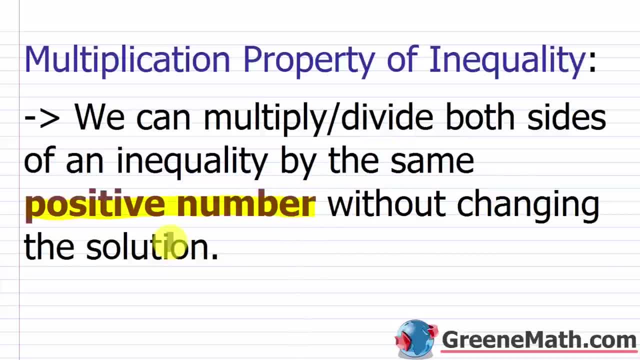 So positive number without changing the solution. 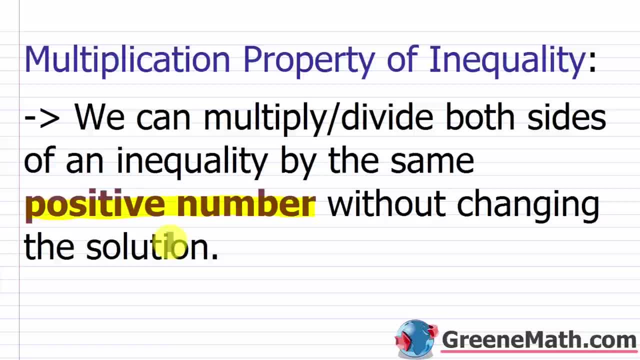 So just like the multiplication property of equality 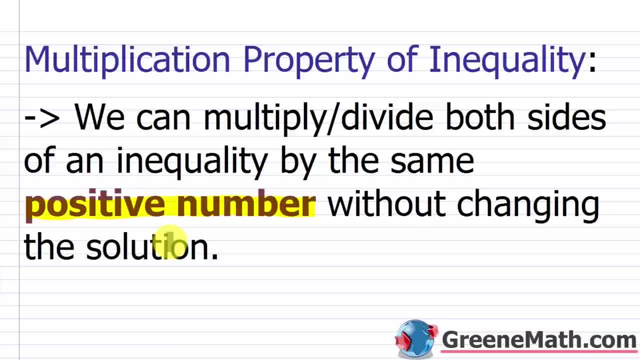 the stipulation there was same non-zero number. 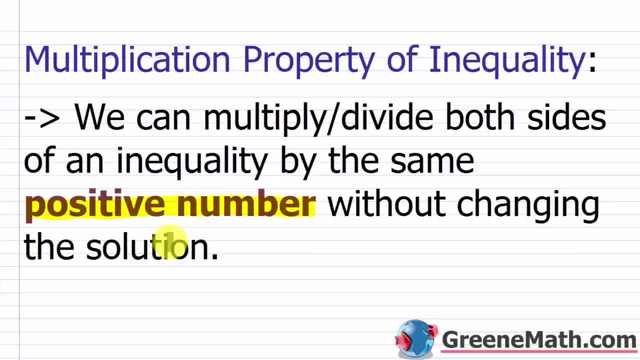 You could multiply both sides of an equation by the same non-zero number and you didn't change the solution. 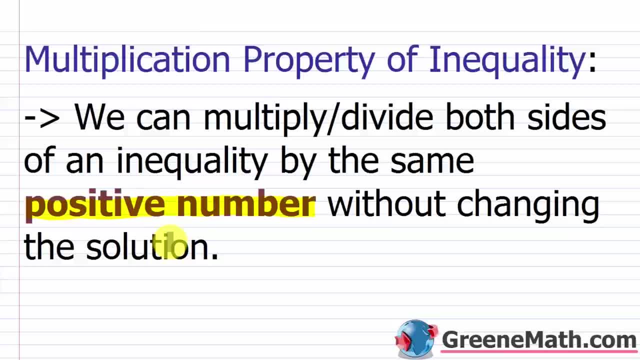 Here what I'm telling you is that you can multiply or divide both sides of an inequality by the same positive number and positive does not include zero. Zero is not positive or negative. It's neither. So by the same positive number without changing the solution. 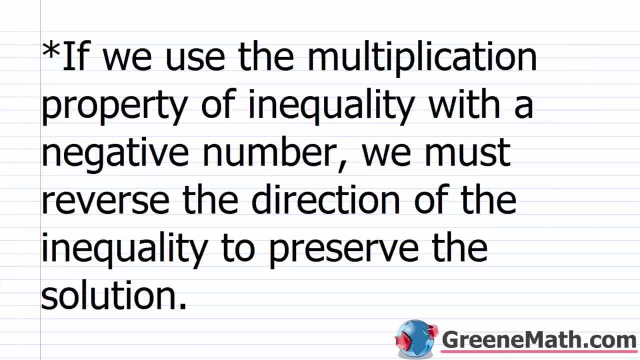 Here's where we run into problems and I can't tell you how many tests I've graded in my life and I've seen students just not get this. 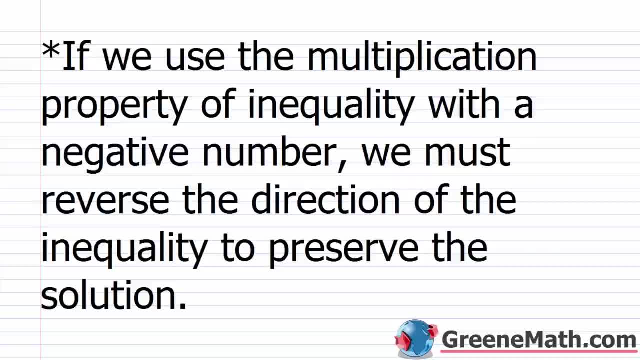 If we use the multiplication property of inequality with a negative number something that is less than zero we must reverse the direction of the inequality to preserve the solution. 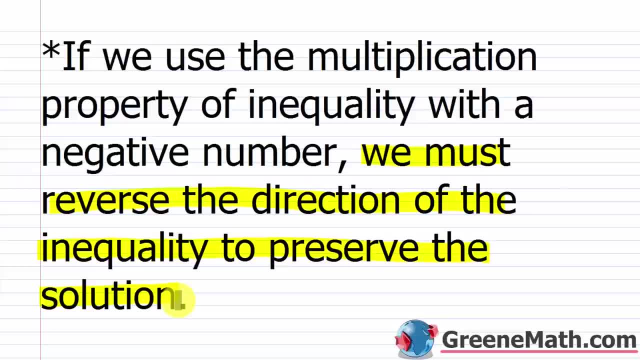 So if you multiply both sides of the inequality by the same negative number flip the inequality. 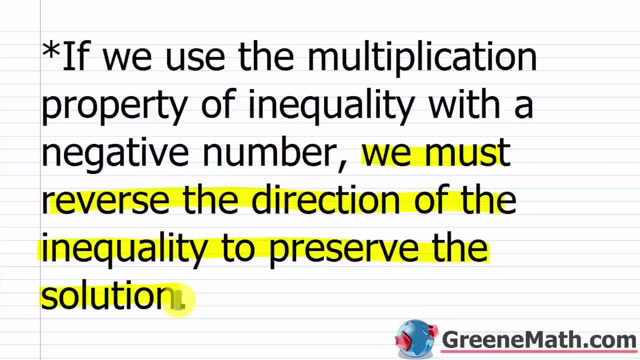 If you divide both sides of the inequality by the same negative number flip the inequality. 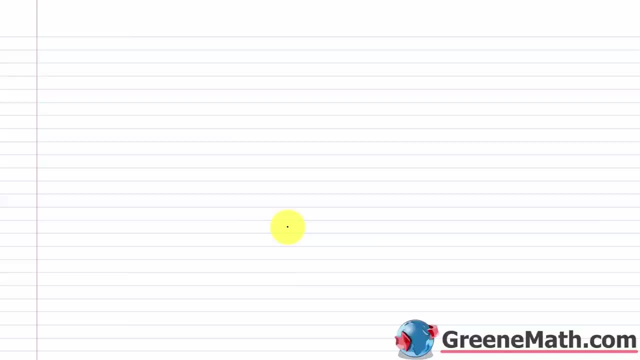 So before we move on and start solving problems let's explore this concept more thoroughly. 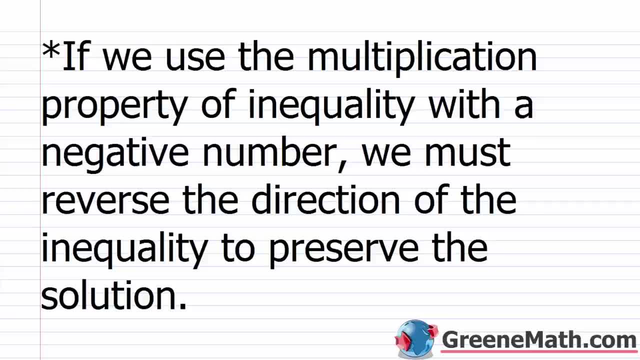 of inequality with a negative number, something that is less than zero. we must reverse the direction of the inequality to preserve the solution. If you multiply both sides of the inequality by the same negative number, flip the inequality. If you divide both sides of the inequality by the same negative number. 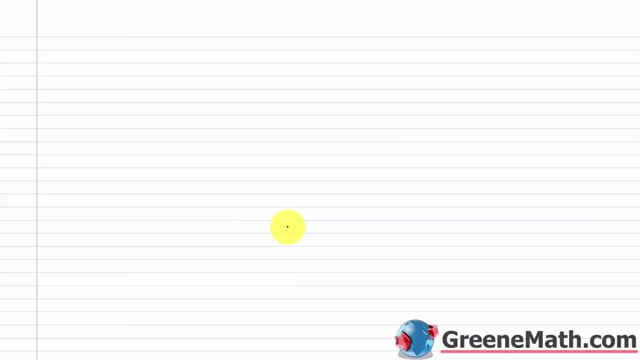 flip the inequality. So before we move on and start solving problems, let's explore this concept more thoroughly. So let's start off with something very, very easy. Let's say I had 2 is less than 7. So at this point we should all know: 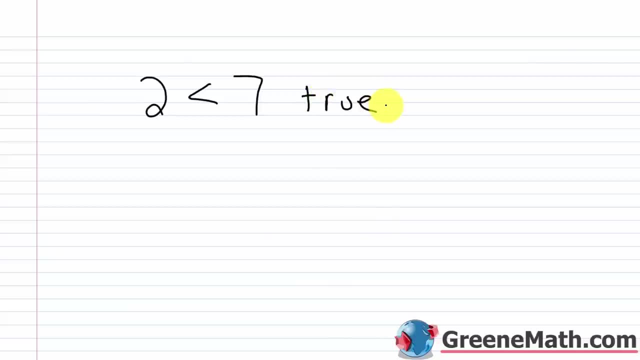 that this is a true statement. A true statement, And what makes it true? Well, 2 is less than 7.. Right 2 is a smaller value than 7.. 2 is to the left of 7 on the number line. 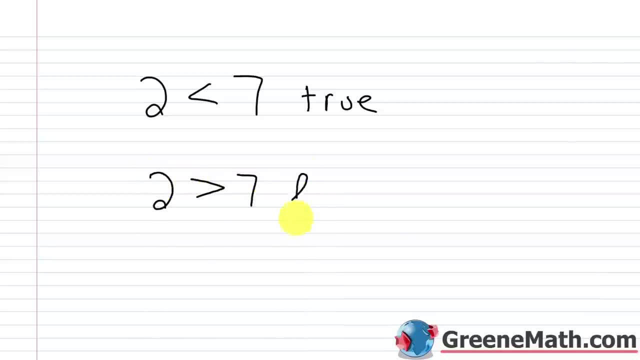 If I had something that said 2 is greater than 7, this would be false. 2 is not greater than 7.. So that's the difference between a true and a false statement when you're dealing with an inequality. So, beginning with a true statement, 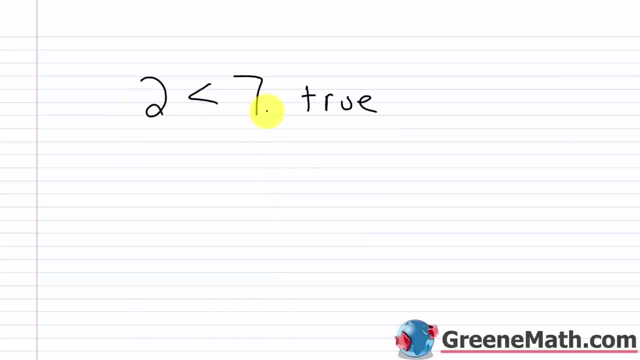 2 is less than 7, we can begin to experiment a little bit. Let's say we think about our multiplication property of inequality And let's say we multiply both sides of the inequality by the same positive number. Recall that this should have no effect. 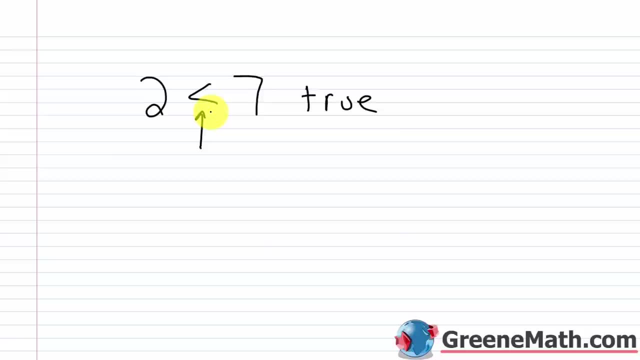 on the direction of the inequality Right. The statement should remain true. So let's say I multiply both sides by the number 4.. So I'll multiply the left by 4 and also the right by 4.. So 4 times 2 is 8.. 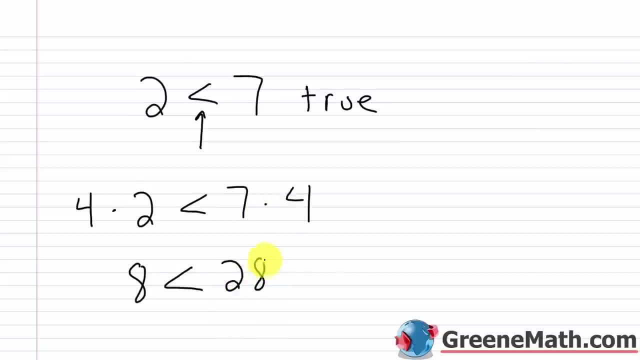 And this should be less than 7 times 4, which is 28.. We can see we still have a true statement. 8 is less than 28.. It's a smaller value. If I have $8 in my pocket, I certainly have less than if I had $28. 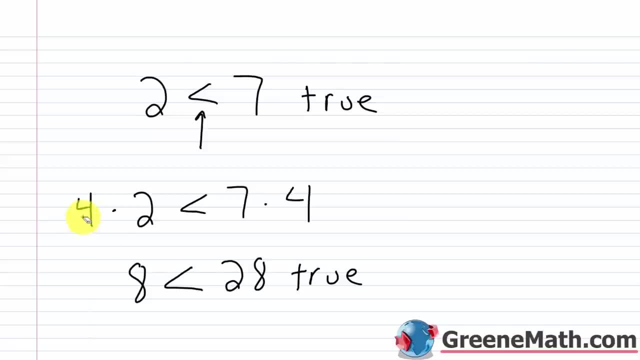 in my pocket. Now let's think about something else Again, starting with this same true statement: let's multiply both sides of the inequality by a negative. now, So let's multiply both sides by negative 4.. Times negative 4 over here. 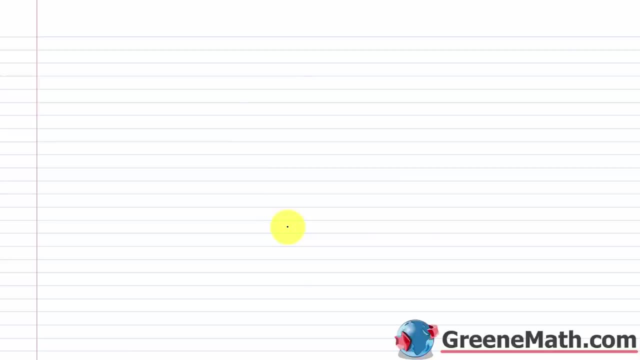 So let's start off with something very very easy. Let's say I had 2 is less than 7. 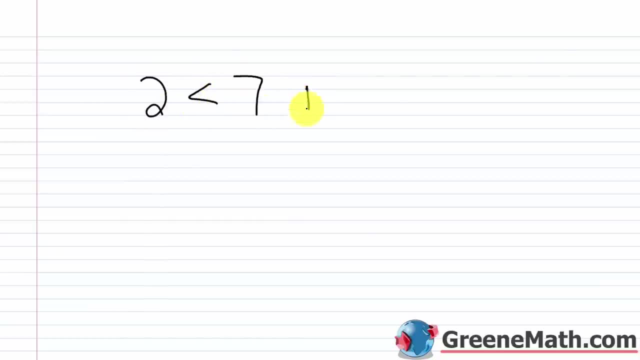 So at this point we should all know that this is a true statement. 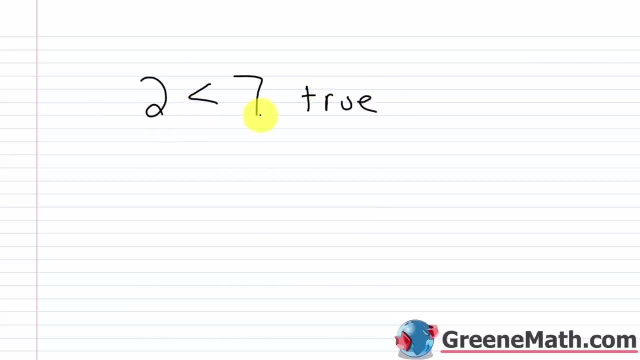 And what makes it true? Well 2 is less than 7. 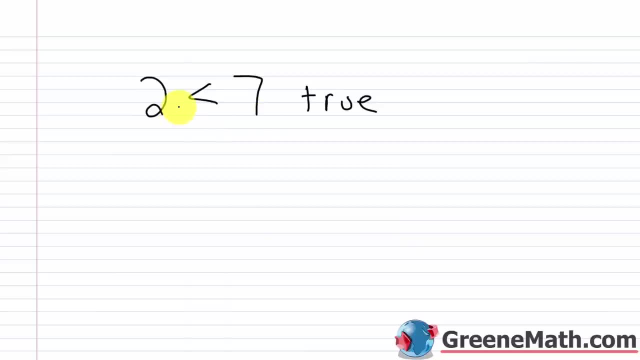 2 is a smaller value than 7. 2 is to the left of 7 on the number line. 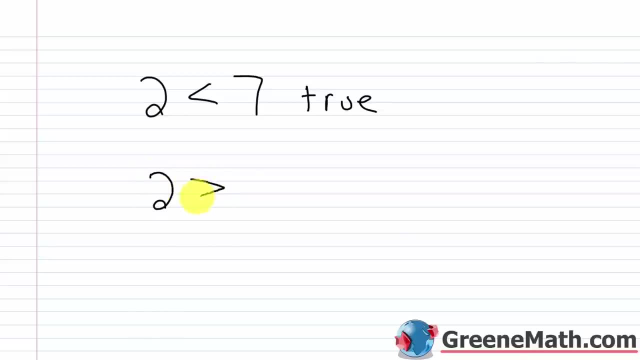 If I had something that said 2 is greater than 7 this would be false. 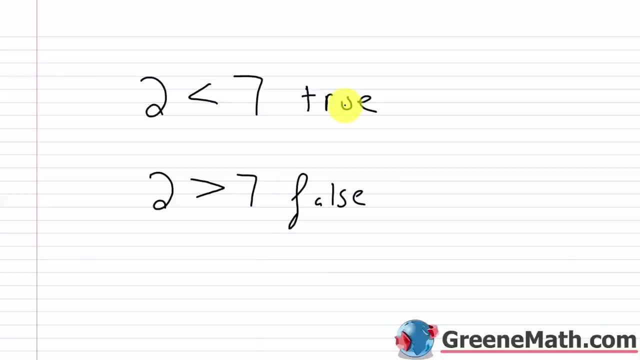 2 is not greater than 7. So that's the difference between a true and a false statement when you're dealing with an inequality. 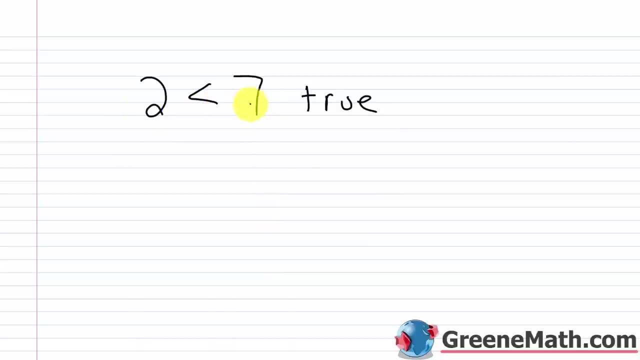 So beginning with a true statement like 2 is less than 7 we can begin to experiment 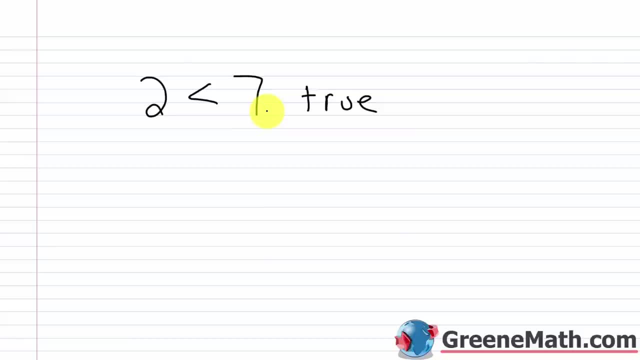 a little bit. Let's say we think about our multiplication property of inequality. 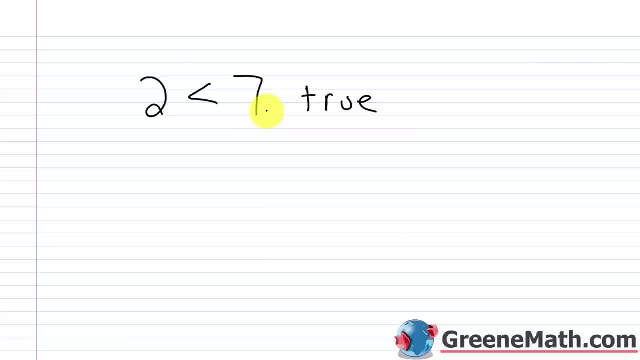 And let's say we multiply both sides of the inequality by the same positive number. Recall that this should have no effect 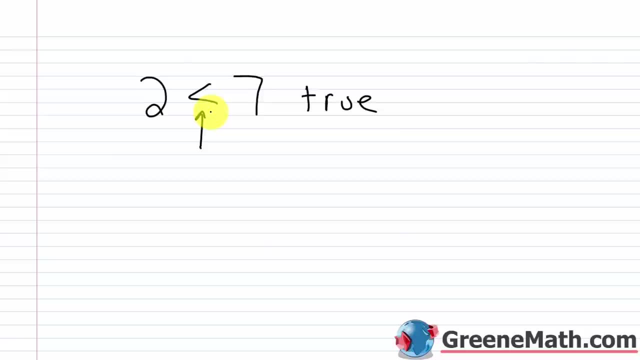 on the direction of the inequality. The statement should remain true. 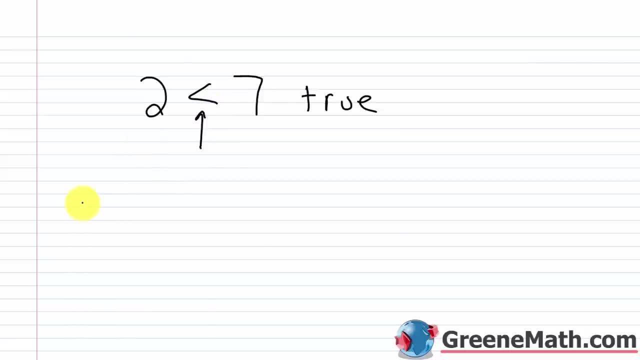 So let's say I multiply both sides by the number 4. So I'll multiply the left by 4 and also the right by 4. 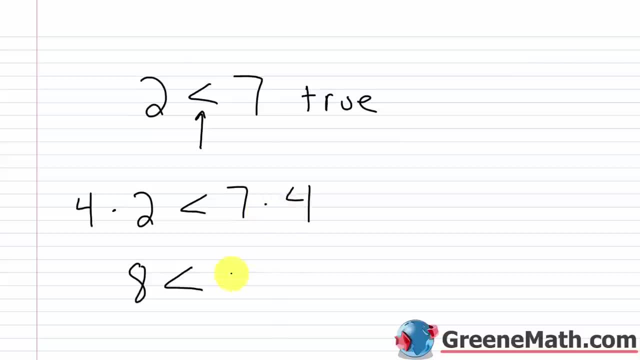 So 4 times 2 is 8 and this should be less than 7 times 4 which is 28. And we can see we still have a true statement. 8 is less than 28. 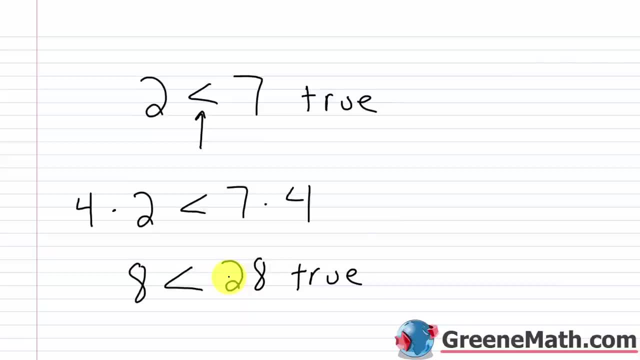 It's a smaller value. If I have $8 in my pocket I certainly have less than if I had $28 in my pocket. Now let's think about something else. 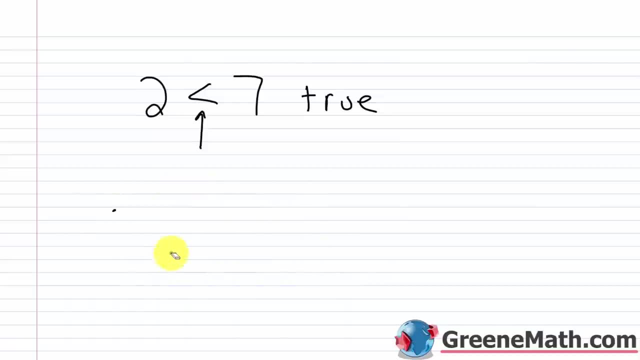 Again starting with this same true statement 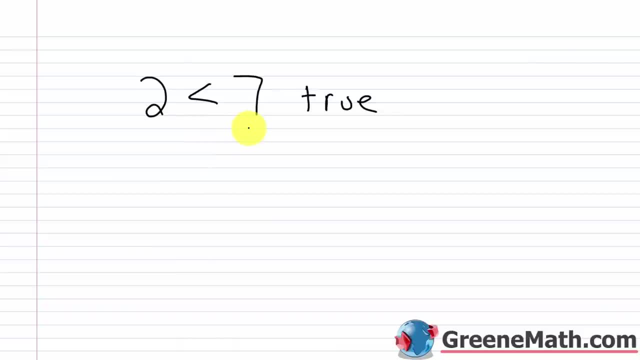 let's multiply both sides of the inequality by a negative now. So let's multiply both sides by 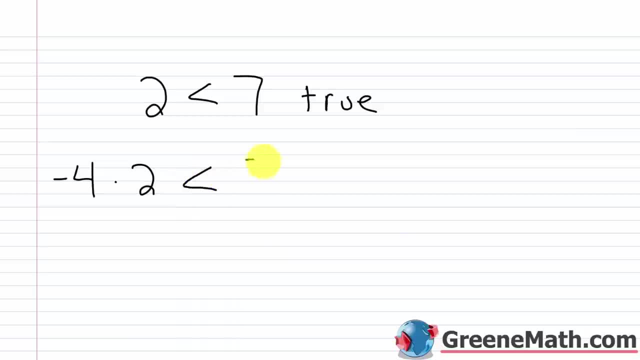 negative 4. So times negative 4 over here and times negative 4 over here. 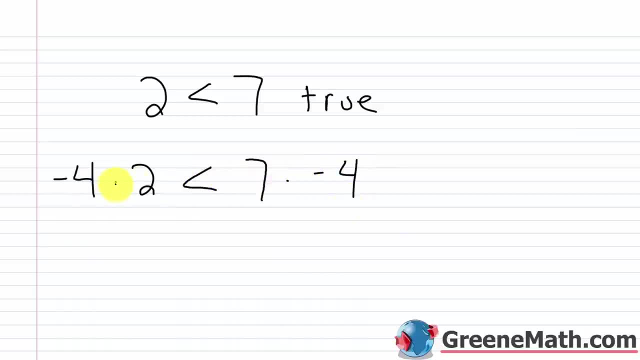 And times negative 4 over here. Now, negative 4 times 2 is now negative 8. And we're saying this is less than 7 times negative 4, which is negative 28.. Now the statement is false And a lot of you. 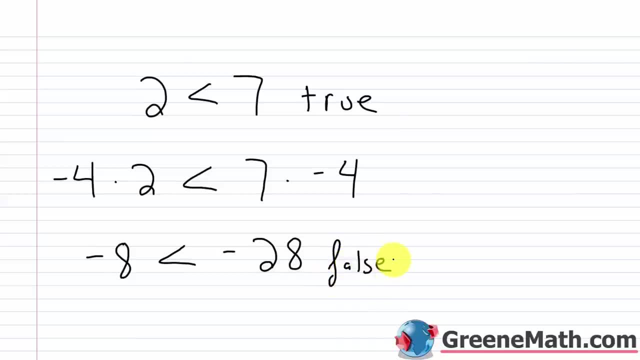 who haven't worked with integers a lot might be a little confused by that. But think about this. for a second, Negative 8 is actually a larger value than negative 28.. Negative 8 is not less than negative 28.. And you kind of think about this. 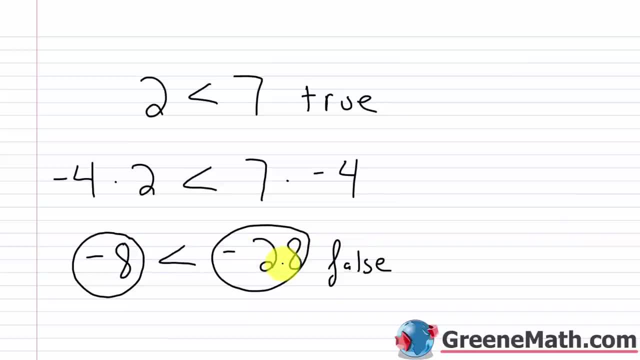 involving the number line. Negative 8 is to the right of negative 28 on the number line. Negative 28 is to the left of negative 8 on the number line. You kind of think about it either way And remember if a number is larger. 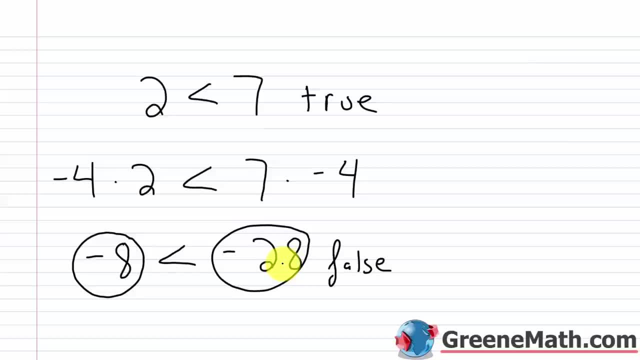 than another, it lies to the right of it on the number line, And if a number is smaller than another, it lies to the left of it on the number line. So this is false. In order for us to get a true statement again, when we multiply both sides by that same negative value, we have to flip the direction of the inequality. 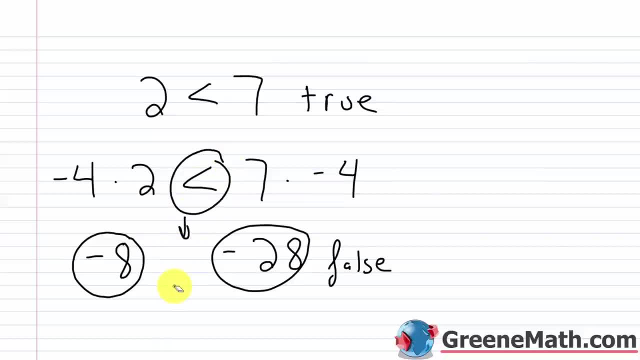 So if I would have flipped this here, instead of a less than now I'd have a greater than. then we could say it's true. Then we could say it's true, right, Negative 8 is greater than negative 28.. 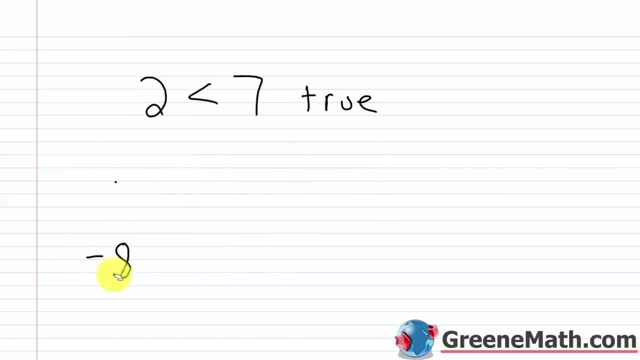 And let me show you one more example of this real quick before we move on. So again, let's start out with a true statement. Let's say I had something like 10 is greater than 5.. So at this point we all know this is true. 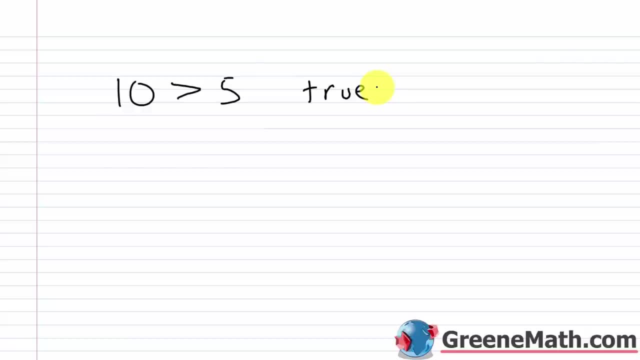 Again, if I multiply both sides by the same positive value, we'll still have a true statement. So let's say we multiply both sides by positive 2.. So positive 2 times 10 is greater than 5 times positive 2.. 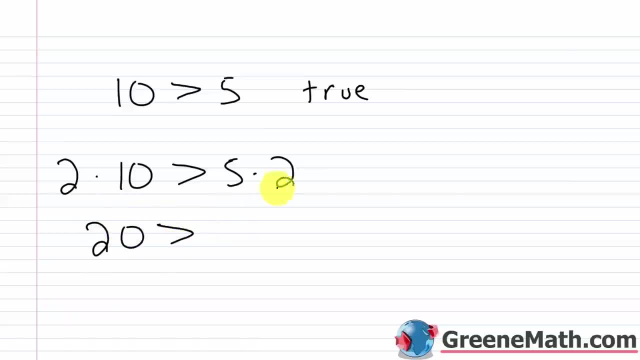 And 2 times 10 is 20.. And this is larger than, or greater than 5 times 2,, which is 10.. Yeah, this is still true, Again, if I multiply both sides by the same negative value. in order for me to keep a true statement, I've got to reverse the direction of the inequality. 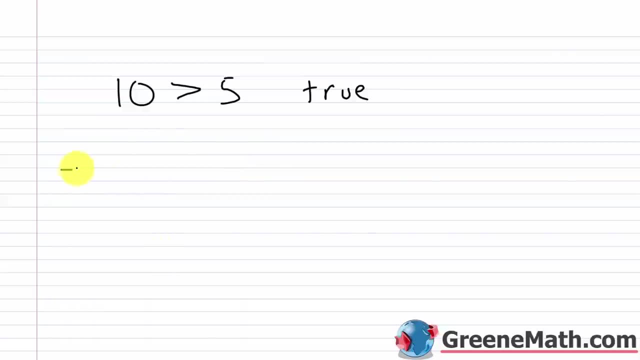 So if we erase this and say, okay, so let's multiply both sides by negative 3.. So let's multiply by negative 3 over here and by negative 3 over here, And we're just going to leave this as it is for now and I'll show you that it's false. 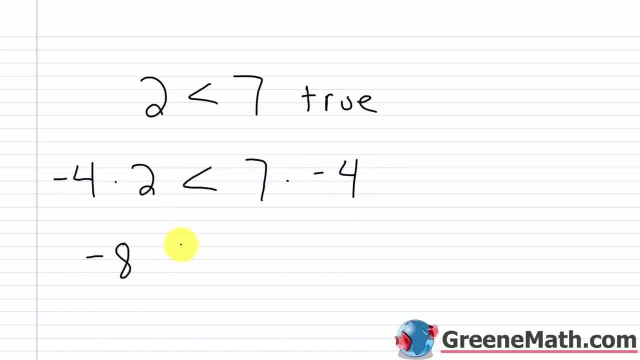 Now negative 4 times 2 is now negative 8. And we're saying this is less than 7 times negative 4 which is negative 28. 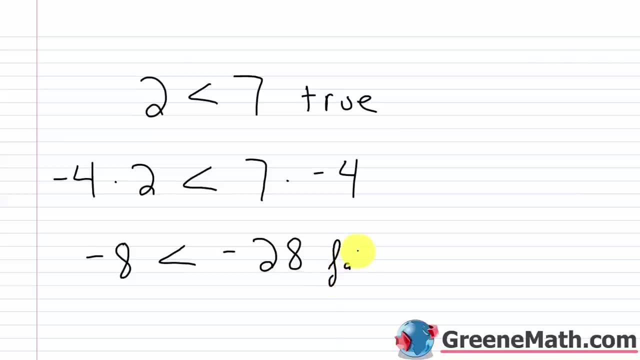 Now the statement is false. And a lot of you who haven't worked with integers a lot might be a little confused by that. 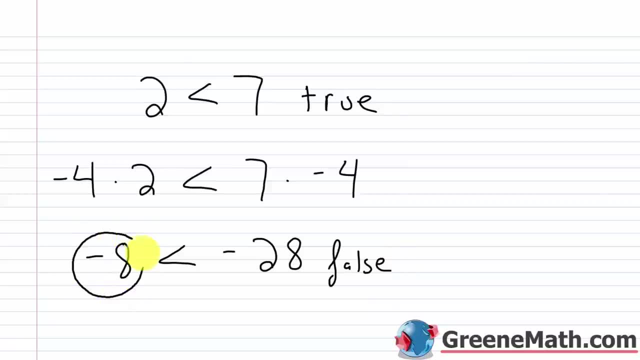 But think about this for a second. Negative 8 is actually a larger value than negative 28. Right? It is not less than negative 28. 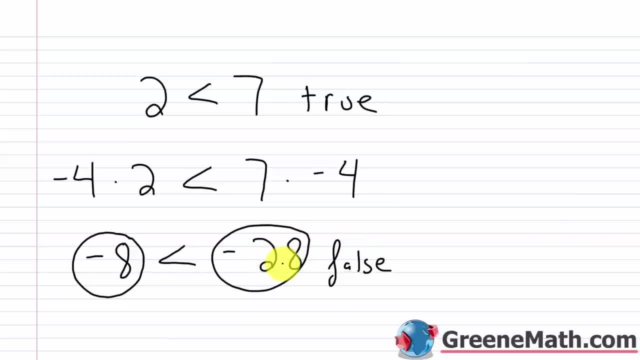 And you kind of think about this involving the number line. 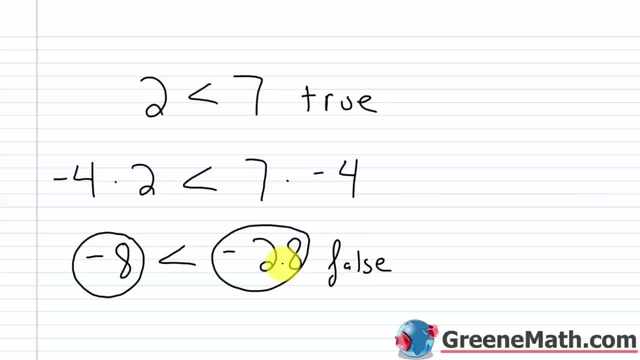 Negative 8 is to the right of negative 28 on the number line. Negative 28 is to the left of negative 8 on the number line. You kind of think about it either way. 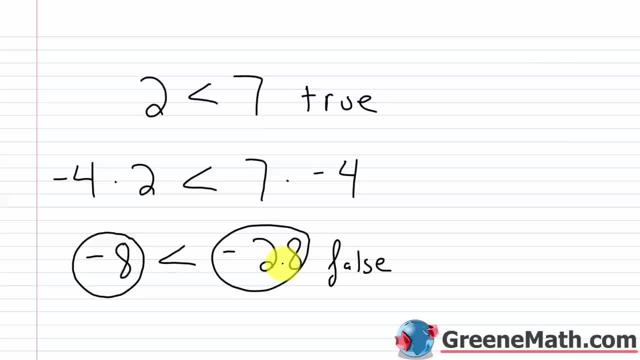 And remember if a number is larger than another it lies to the right of it on the number line. 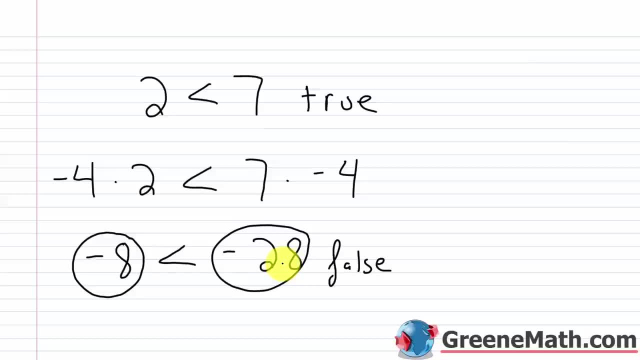 And if a number is smaller than another it lies to the left of it on the number line. So this is false. In order for us to get a true statement again when we multiply both sides by that same negative value we have to flip the direction of the inequality. So if I would have flipped this here instead of a less than now I'd have a greater than then we could say it's true. Then we could say it's true. Right? 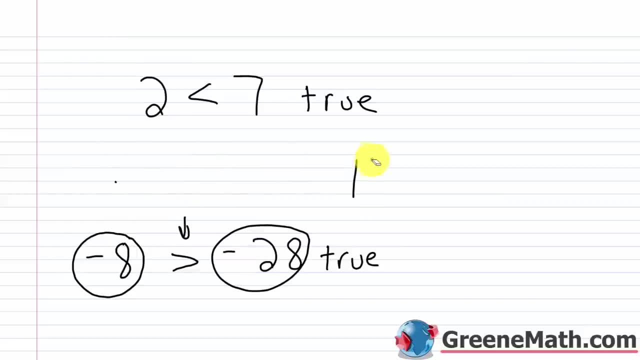 Negative 8 is greater than negative 28. And let me show you one more example of this real quick before we move on. 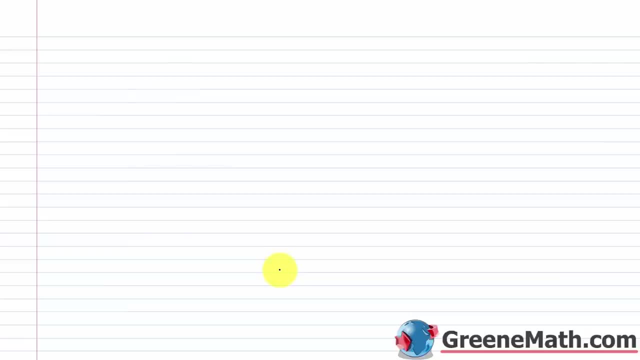 So again let's start out with a true statement. Let's say I had something like 10 is greater than 5. So at this point we all know this is true. 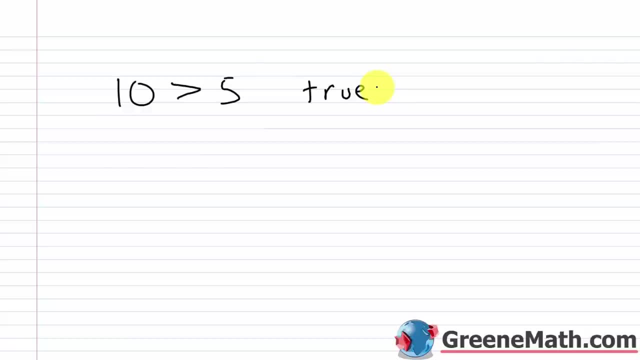 Again if I multiply both sides by the same positive value we'll still have a true statement. 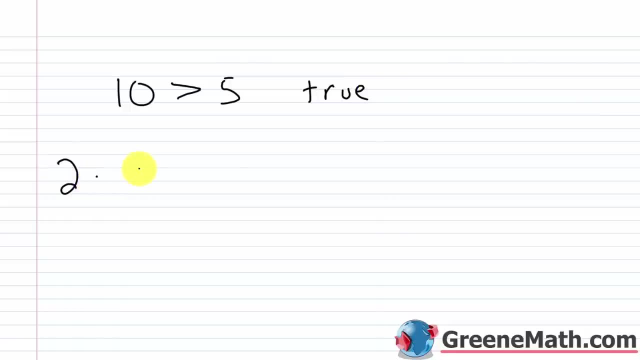 So let's say we multiply both sides by positive 2. So positive 2 times 10 is greater than 5 times positive 2. And 2 times 10 is 20. And this is larger than or greater than 5 times 2 which is 10. 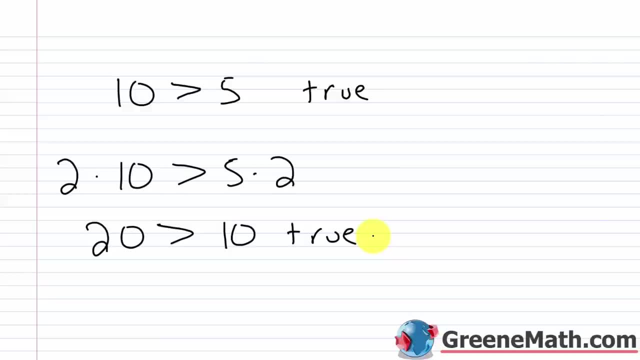 Yeah this is still true. Again if I multiply both sides by the same negative value in order for me to keep a true statement I've got to reverse the direction of the inequality. So if we erase this and say okay let's multiply both sides by negative 3. So let's multiply by negative 3 over here. And by negative 3 over here. And we're just going to leave this as it is for now and I'll show you that it's false. Negative 3 times 10 is negative 30. And we're saying this is greater than 5 times negative 3 which is negative 15. And again now this is false. 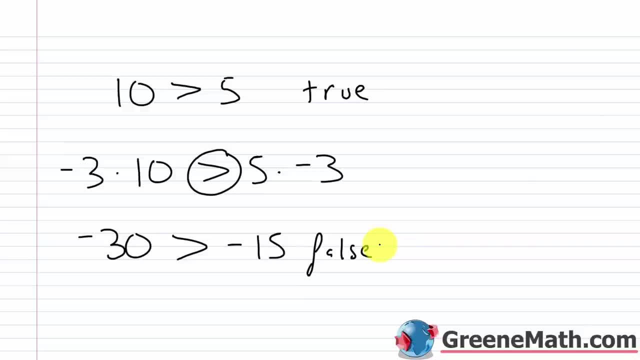 Right? It doesn't work anymore. And one of the reasons you can kind of think about this is okay if I'm starting out with a bigger number when I multiply it by a negative I'm going to have a bigger negative and a bigger negative is actually a smaller number. Right? As numbers go this way. As the numbers get bigger and bigger in the negative direction they're actually getting smaller. And I know again if you haven't had a lot of experience kind of thinking about integers in that way it might be a little confusing but just think about 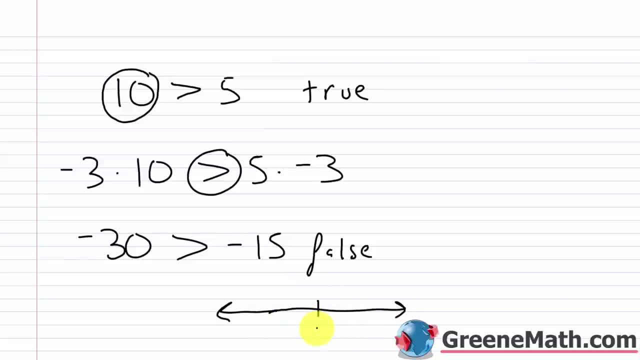 your number line. Right? It looks like this. Here's 0. And as numbers move this way. Right? You're getting smaller and smaller values. 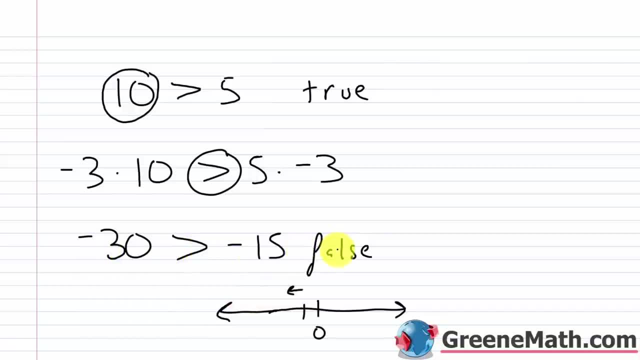 So in this case negative 30 is greater than negative 15 would be false. In order for us to have gotten a true statement when we multiplied both sides by the same negative value we have to flip. 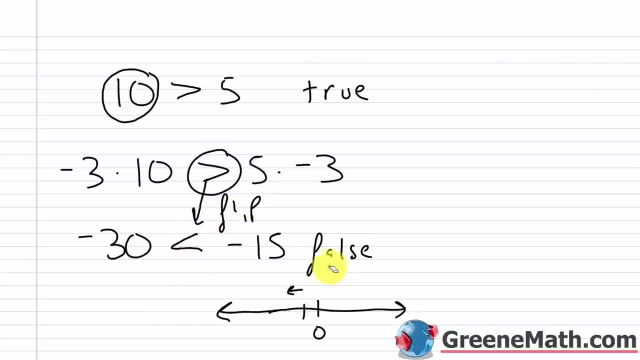 We have to flip. And so this would be a less than and that would make it a true statement. 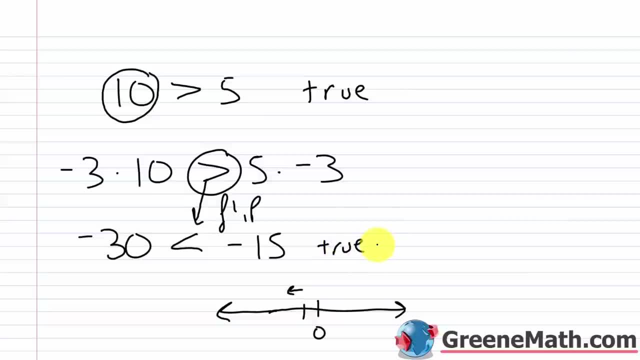 So just keep that in mind as you're working these problems. 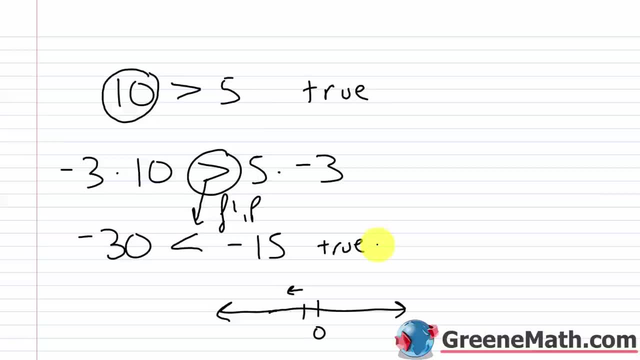 Again if you multiply or divide by the same negative value you've got to flip the direction of the inequality in order to get the correct answer. 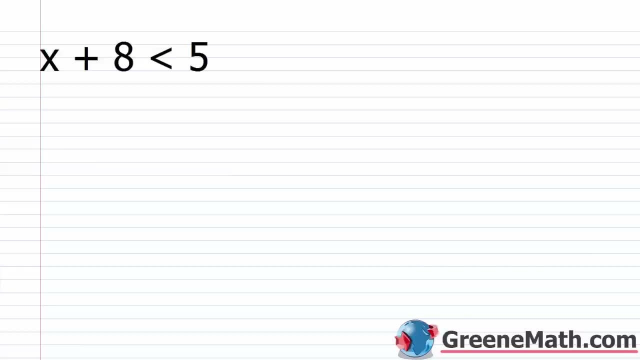 Alright let's take a look at some sample problems. And we're going to use the same skill set we used from equations. Our goal is always to isolate x. Whether we're solving an inequality or an equation. And again we use kind of the same techniques here. So I have x plus 8 is less than 5. I want to isolate my variable x. So I want to isolate this guy. 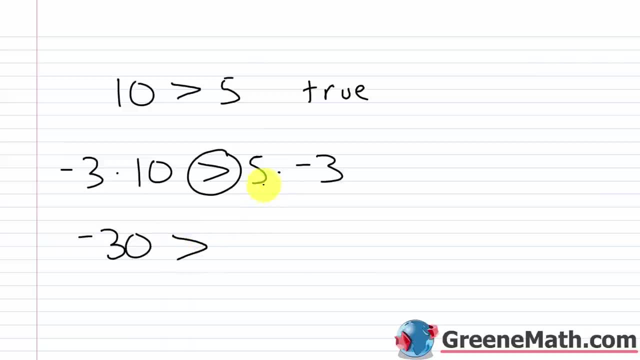 Negative 3 times 10 is negative 30. And we're saying this is greater than 5 times negative 3, which is negative 15.. And again, now this is false, right, It doesn't work anymore, And one of the reasons you can kind of think about this is: okay. 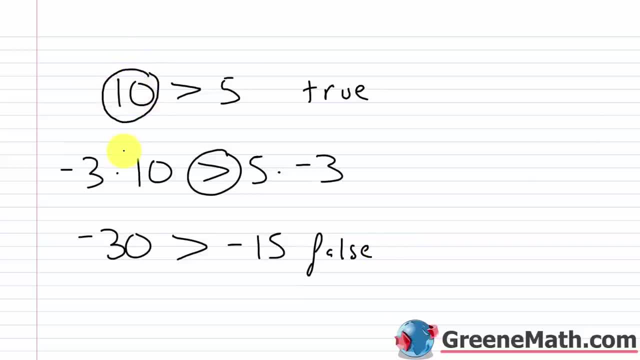 if I'm starting out with a true statement, I'm going to have to reverse the direction of the inequality. If I'm starting out with a bigger number, when I multiply it by a negative, I'm going to have a bigger negative, and a bigger negative is actually a smaller number, right? 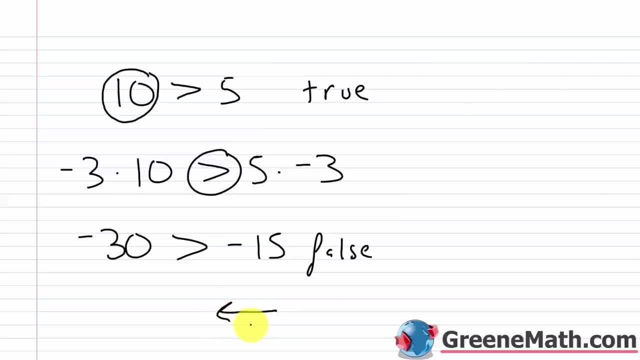 As numbers go this way, as the numbers get bigger and bigger in the negative direction, they're actually getting smaller. And I know again, if you haven't had a lot of experience kind of thinking about integers in that way, it might be a little confusing. but just think about your number line, right? 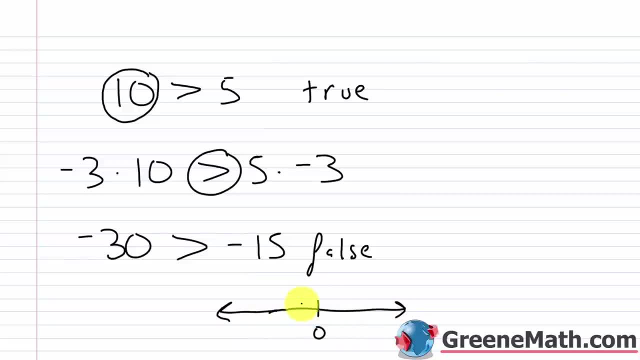 It looks like this: Here's 0. And as numbers move this way, right, you're getting smaller and smaller values. So in this case, negative 30 is greater than negative 15 would be false In order for us to have gotten a true statement. 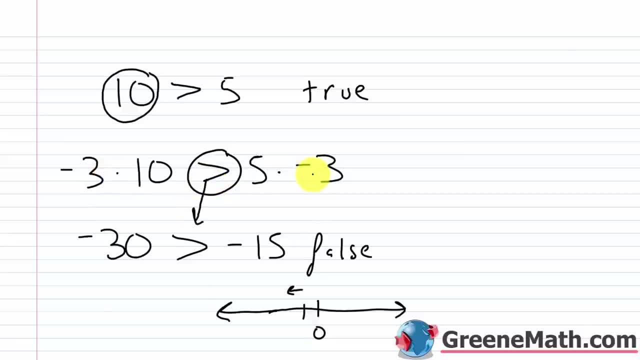 when we multiply both sides by the same negative value, we have to flip, We have to flip, And so this would be a less than, and that would make it a true statement. So just keep that in mind as you're working these problems. 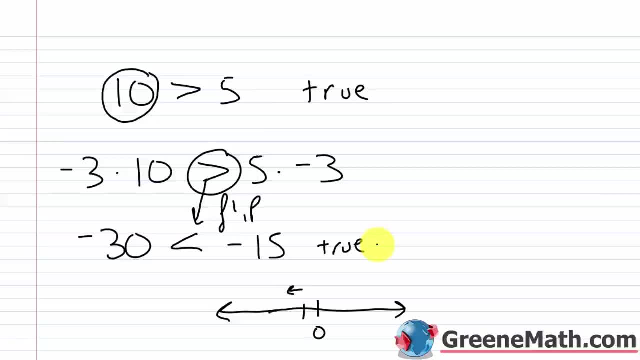 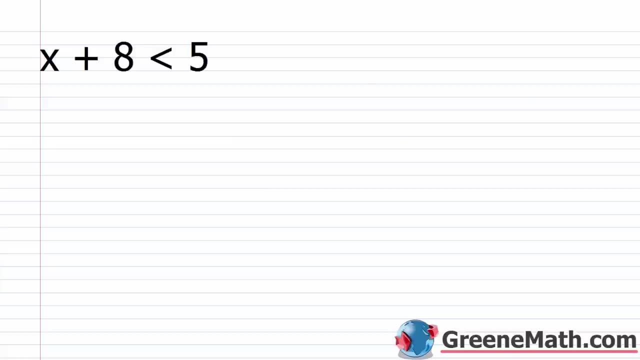 Again, if you multiply or divide by the same negative value, you've got to flip the direction. You've got to flip the direction of the inequality in order to get the correct answer. All right, let's take a look at some sample problems. 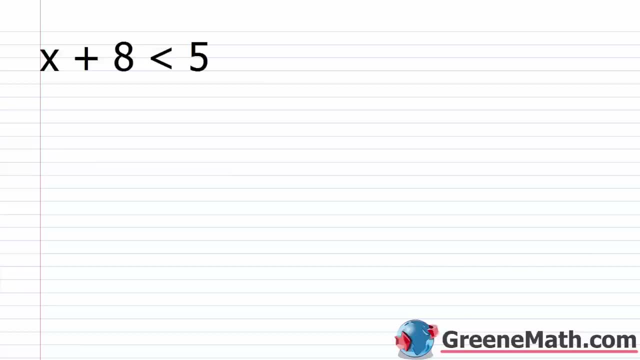 And we're going to use the same skill set we used from equations. Our goal is always to isolate x, whether we're solving an inequality or an equation, And again we use kind of the same techniques here. So I have: x plus 8 is less than 5.. 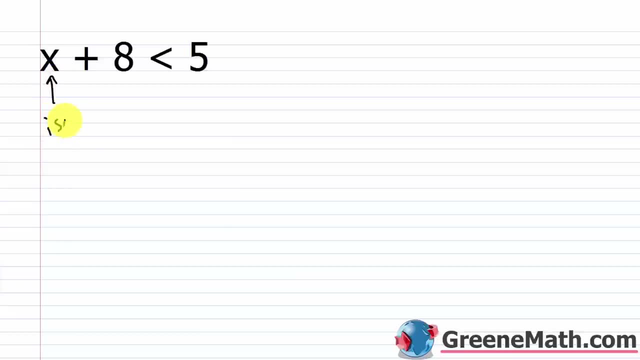 I want to isolate my variable x, So I want to isolate this guy. So all I need to do in this case is is move 8 away. So to do that, I just subtract 8 from both sides of the inequality. So minus 8,, minus 8.. 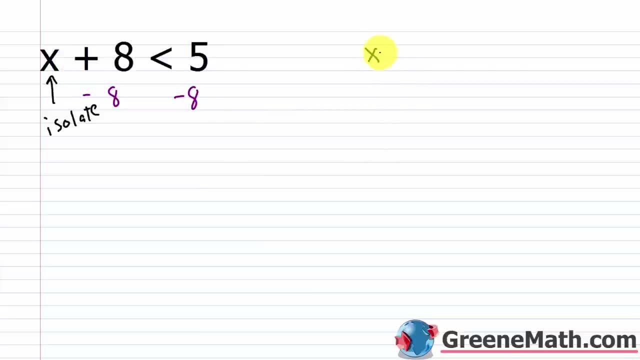 Very, very simple. Remember when we're solving equations like x plus 8 equals 5, I did the same thing. I just subtracted 8 away from each side and I got a solution: of x is equal to negative 3.. 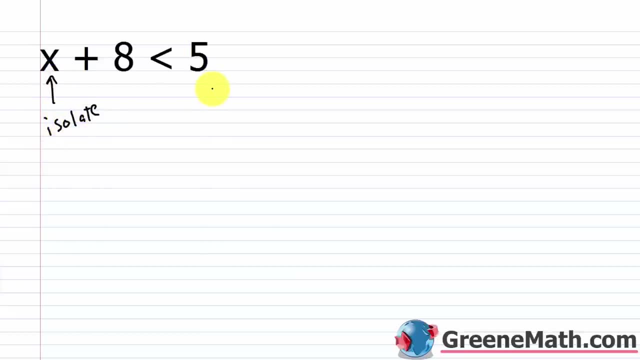 So all I need to do in this case is move 8 away. So to do that I just subtract 8 from both sides of the inequality. So minus 8 minus 8. Very very simple. Remember when we were solving equations like x plus 8 equals 5. I did the same thing. I just subtracted 8 away from each side. And I got a solution of x is equal to negative 3. 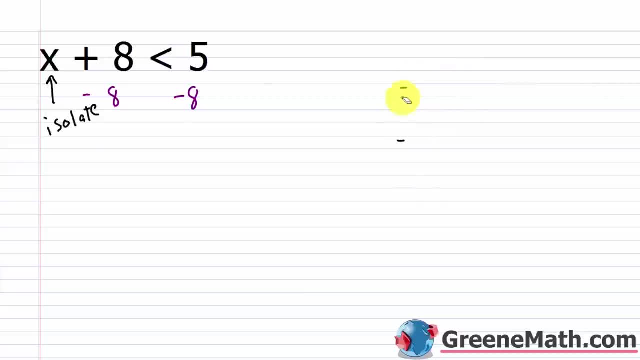 Well it's the same. I'm just isolating x and I'm using pretty much the same techniques. 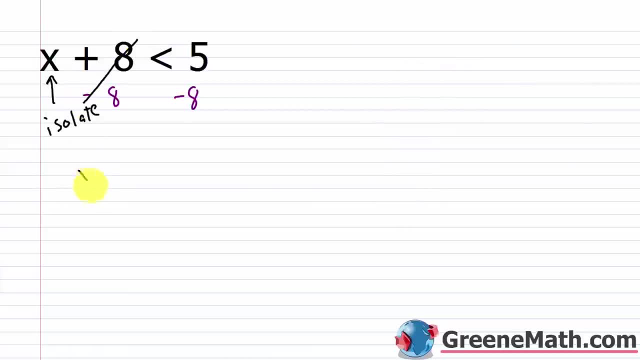 So this will cancel. x is now isolated. 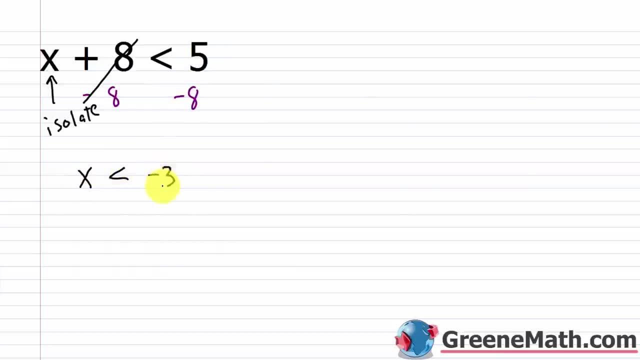 And it's less than 5 minus 8 is negative 3. So what we're saying is that x can be any number that is less than negative 3 and I'll get a true statement. 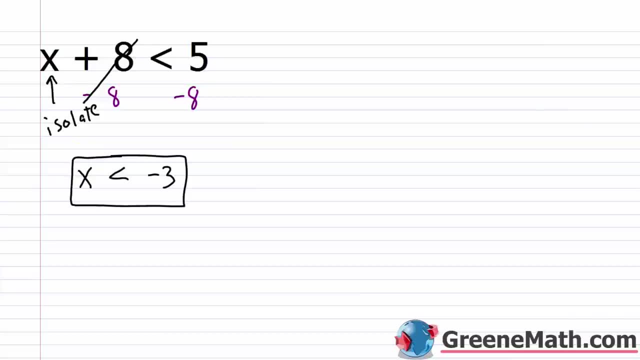 Alright so let's write our solution using interval notation. And in most cases this is what your teacher is going to expect you to do. So the smallest value that x can take on is really negative infinity. Right because x can be anything less than negative 3. So we'll write negative infinity. 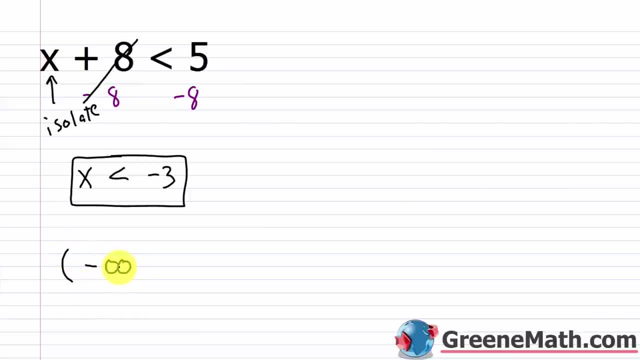 And remember we put a parenthesis next to that because it's not included. 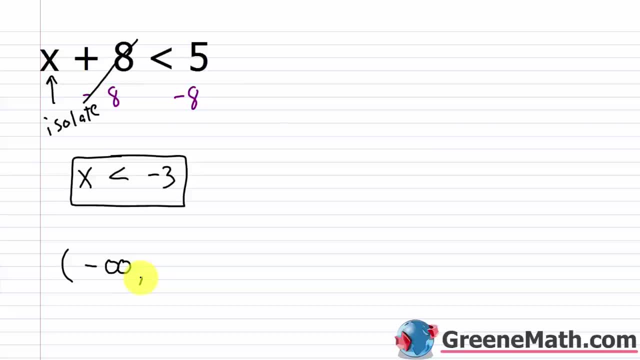 Comma. And then what's the largest value x can take on? Well it's got to be 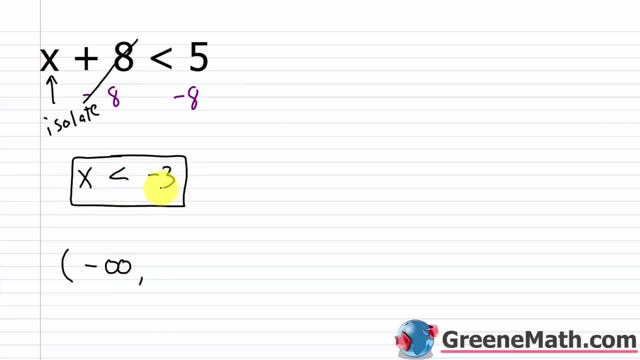 less than negative 3. So it can be any value up to but not including negative 3. So we'll put negative 3 there. And then again we'll put a parenthesis there to say that negative 3 is not included. 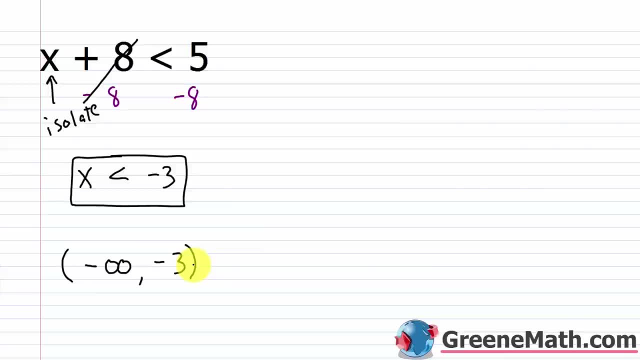 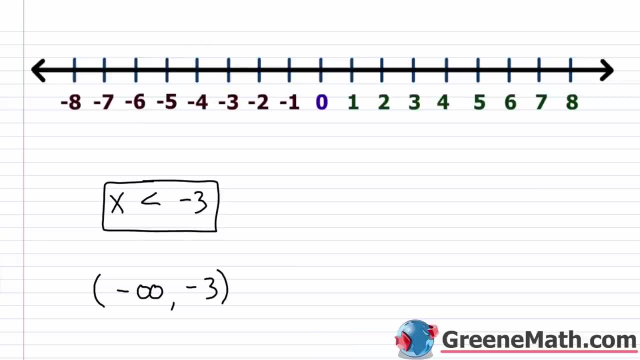 So let's graph this real quick. I'm going to take these down here. And graphically x is less than negative 3. You find negative 3 on your number line. I'm going to put a parenthesis facing to the left. And then I'm going to shade everything this way including that arrow. So this is x is less than negative 3 graphically. 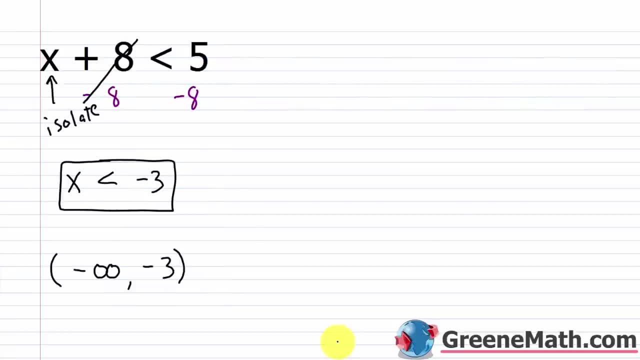 Now when we solved our linear equations in one variable we always checked to make sure that we got the right answer. Checking a linear inequality in one variable is a lot more work. So the official way that you're going to check it is basically to use three steps. So the first thing you're going to do is you're going to replace your 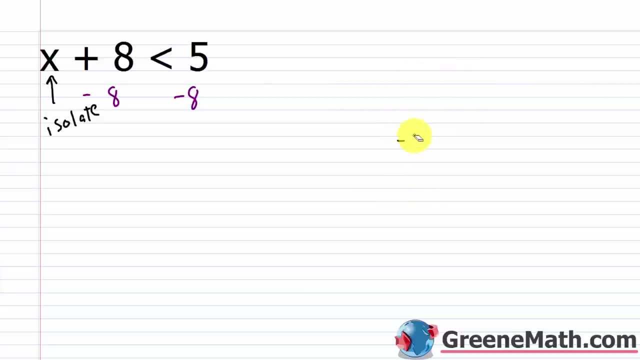 Well, it's the same. I'm just isolating x and I'm using pretty much the same techniques, So this will cancel. x is now isolated And it's less than 5 minus 8 is negative 3.. So what we're saying is that x can be any number that is less than negative 3,. 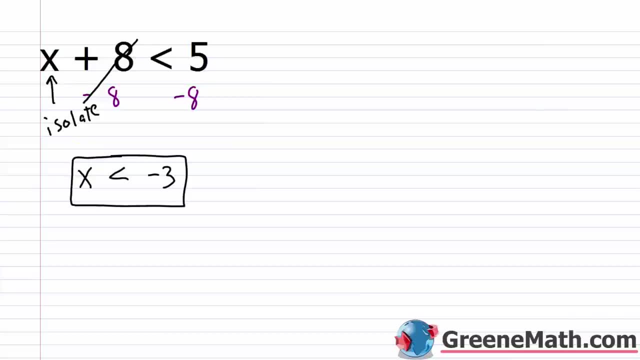 and I'll get a true statement. All right, so let's write our solution using interval notation, And in most cases, this is what your teacher is going to expect you to do. So the smallest value that x can take on is really negative infinity right. 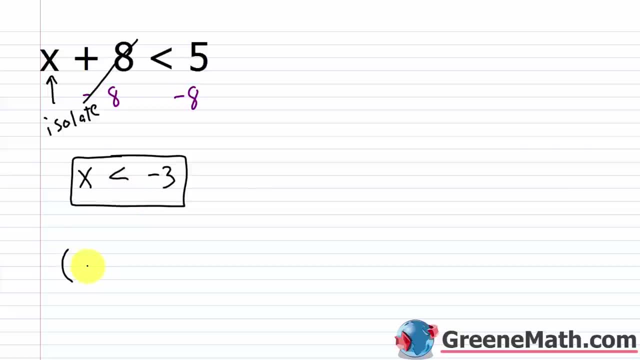 Because x can be anything less than negative 3. So we'll write negative infinity And remember we put a parenthesis. We'll put a parenthesis next to that because it's not included comma. And then what's the largest value x can take on? 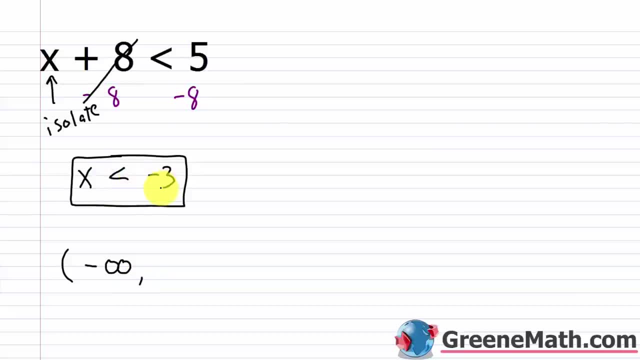 Well, it's got to be less than negative 3.. So it can be any value up to, but not including negative 3.. So we'll put negative 3 there And then again we'll put a parenthesis there to say that negative 3 is not included. 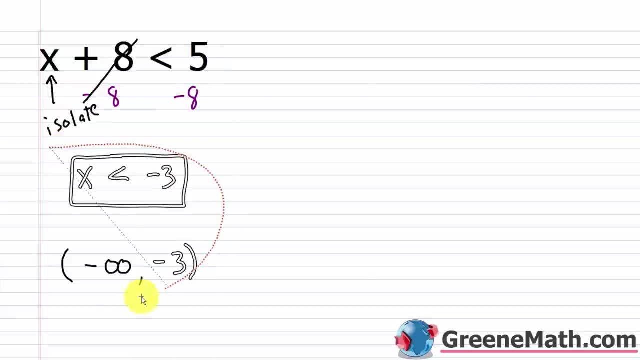 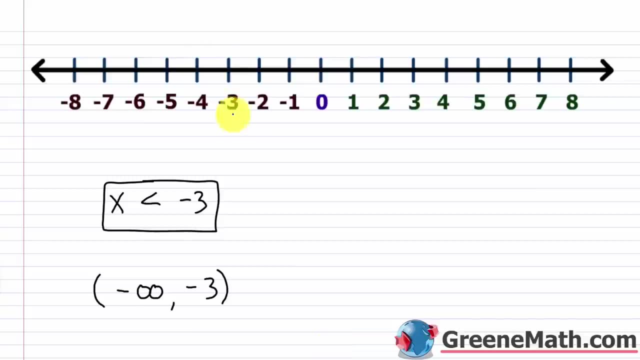 So let's graph this real quick. I'm going to take these down here And graphically, x is less than negative 3.. You find negative 3 on your number line. I'm going to put a parenthesis. facing to the left. 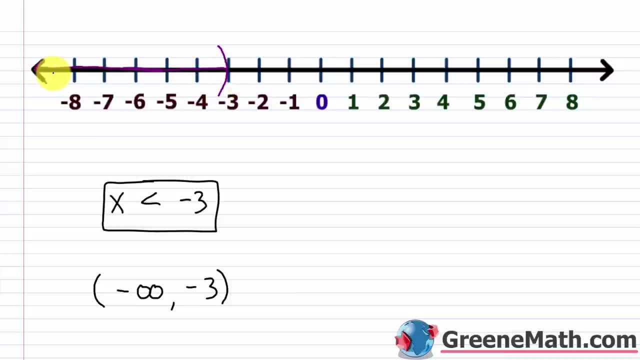 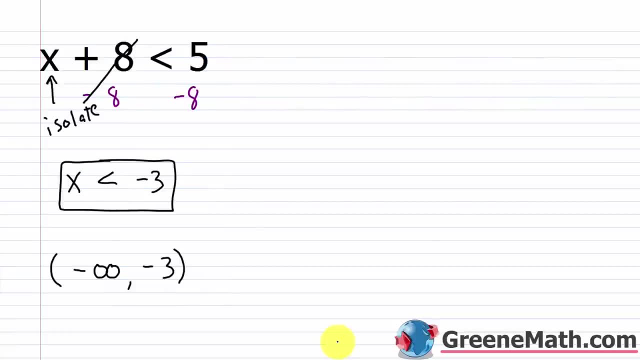 And then I'm going to shade everything this way, including that arrow. So this is: x is less than negative 3 graphically. Now, when we solved our linear equations in one variable, we always checked to make sure that we got the right answer. 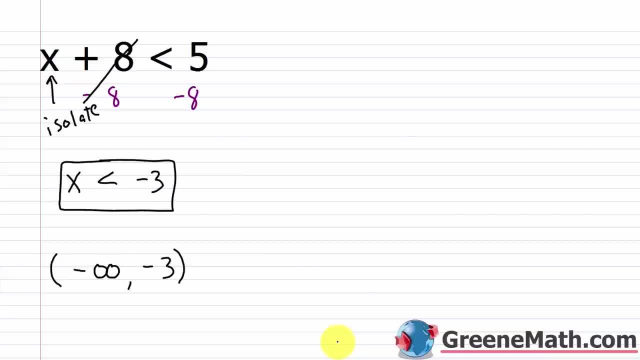 Checking a linear inequality in one variable is a lot more work. So the official way that you're going to check it is basically to use three steps. So the first thing you're going to do is you're going to replace your inequality symbols with equal symbols. 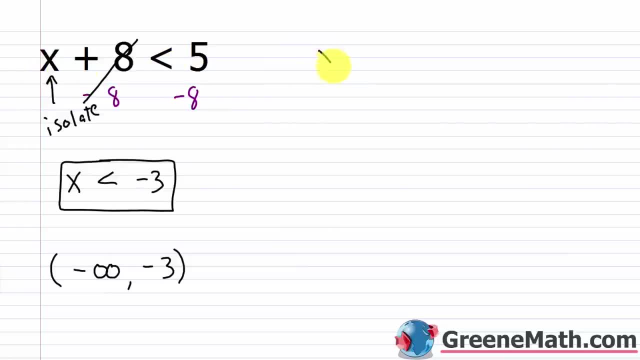 So I'm going to change this: x plus 8 is less than 5 to x plus 8 equals 5.. And I'm going to change: x is less than negative 3 to x equals negative 3.. So I'm going to make sure that this is the solution. 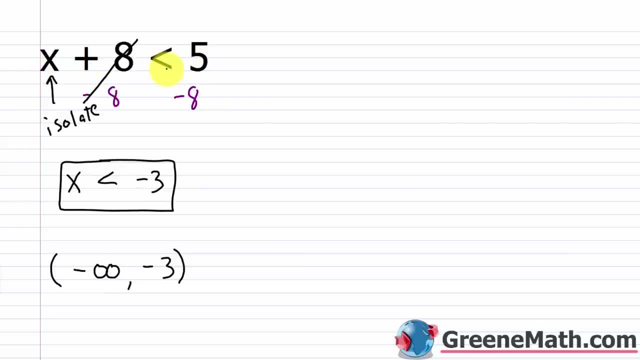 inequality symbols with variable symbols. So I'm going to change this x plus 8 is less than 5 to x plus 8 equals 5. 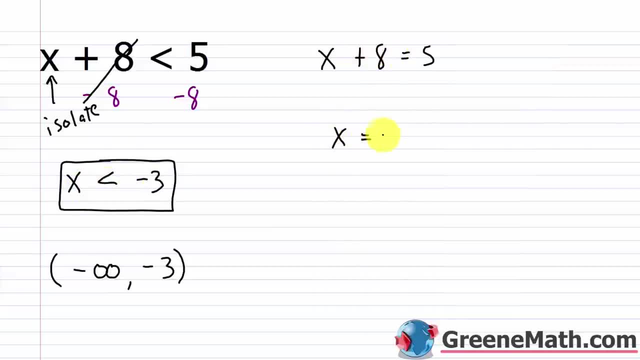 And I'm going to change x is less than negative 3 to x equals negative 3. 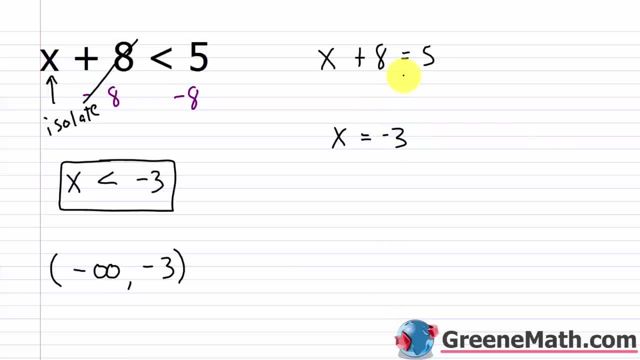 So I'm going to make sure that this is the solution. 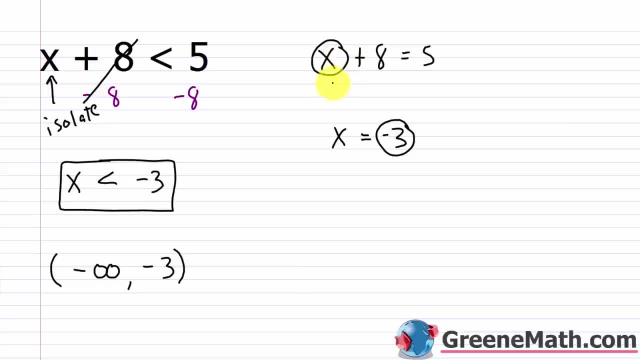 So I'm going to take this negative 3 and plug it in for x. So negative 3 plus 8 does equal 5. So that checks out. 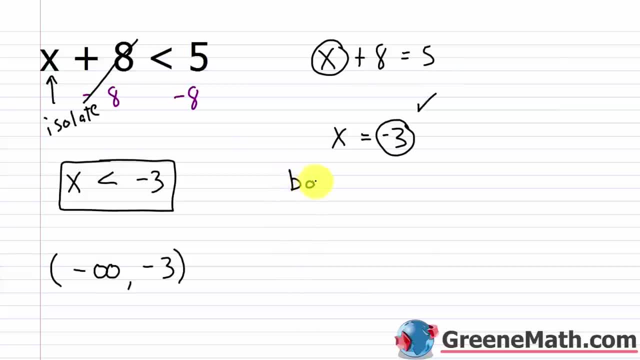 So this is referred to as our boundary. 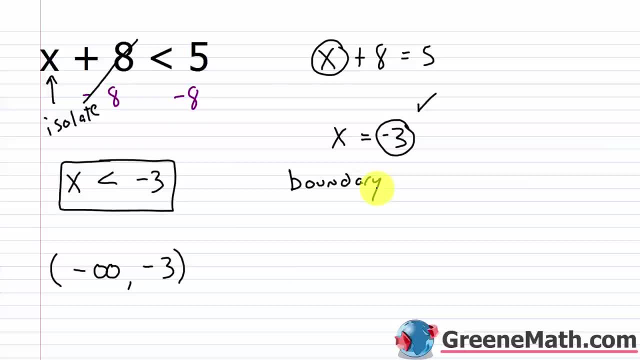 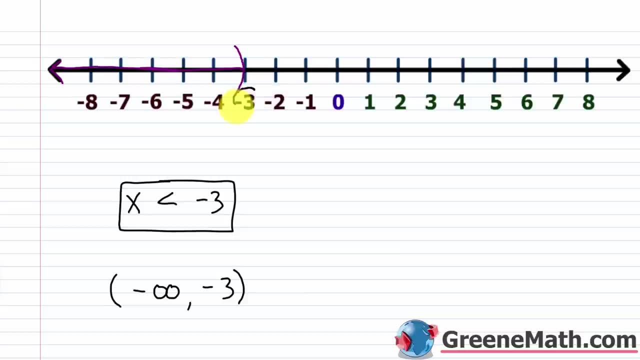 Now the boundary is going to separate the solution region from the non-solution region. And graphically you can kind of see that negative 3 is the cut off. Anything less than negative 3, anything over 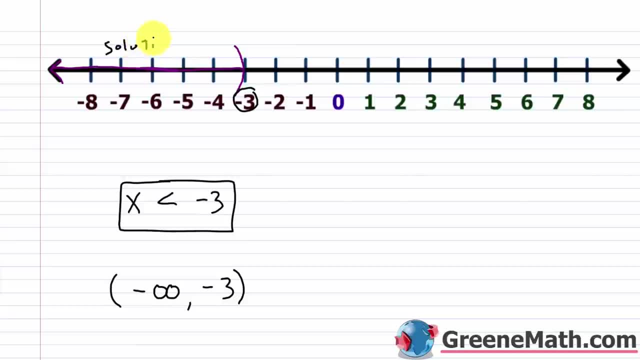 here works. So this is your solution region. 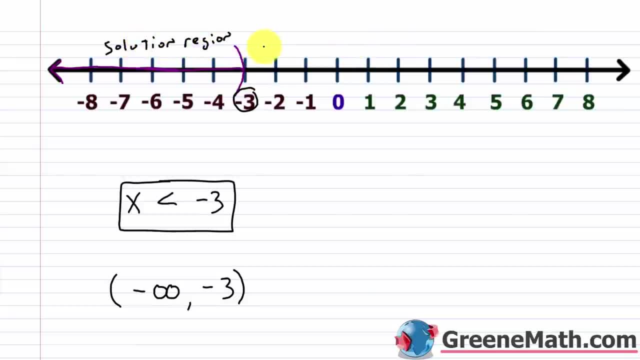 Then anything starting at negative 3 and beyond doesn't work. So this is your non-solution region. 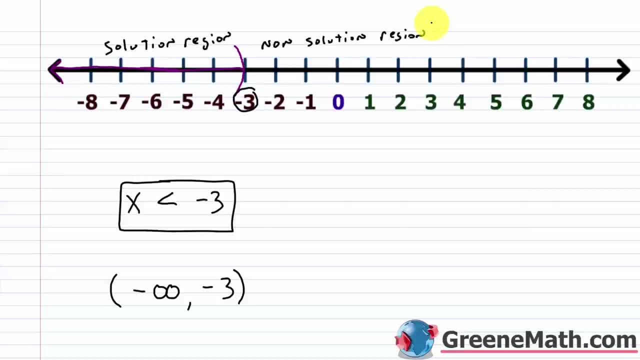 So what we need to do after we establish the boundary we need to take a number from the non-solution region and try it. And then also a number from the solution region and try it. 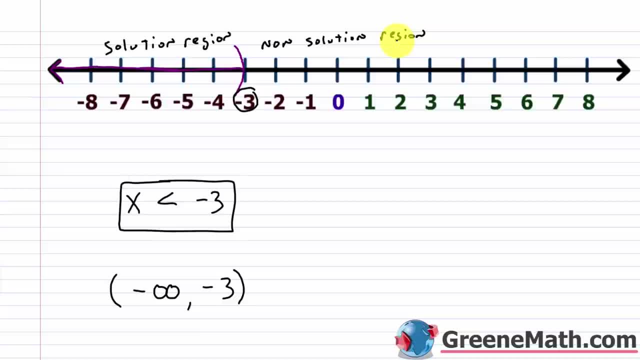 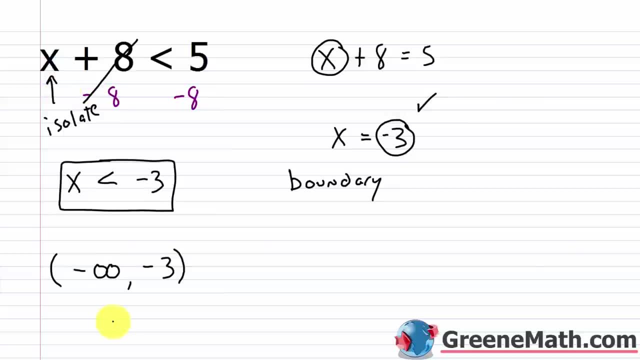 So from the non-solution region the easiest number to try is 0. So let's go back up here and we can plug in a 0 for x and we'd have 8 is less than 5. So that's in the non-solution region so it should be false and it is. 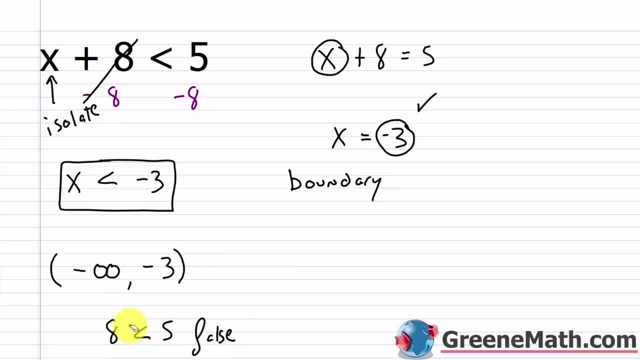 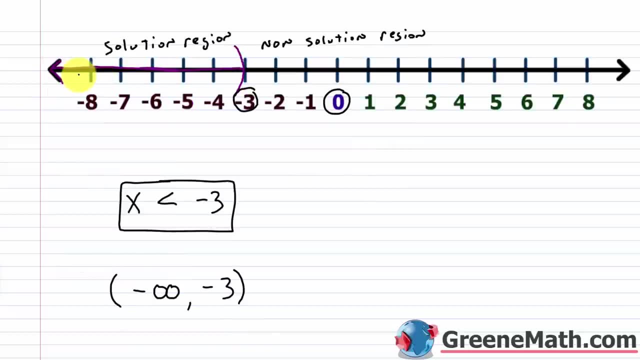 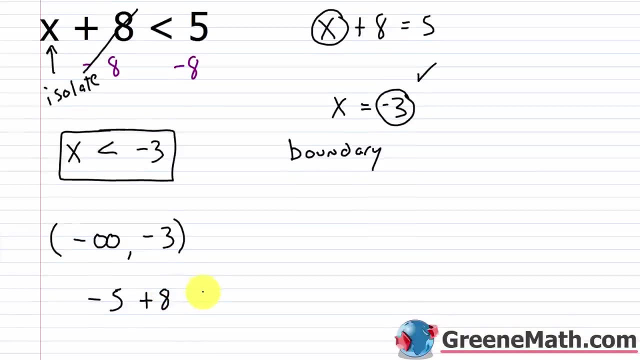 So it's okay that this is false. That's what we want. Now the next thing we're going to do is we're going to pick a number from the solution region. So that's over here. That's anything less than negative 3. So I can pick anything I want. So let's say negative 5. So I'd plug a negative 5 in for x. I'd have negative 5 plus 8 is less than 5. Negative 5 plus 8 is 3 and 3 is less than 5. 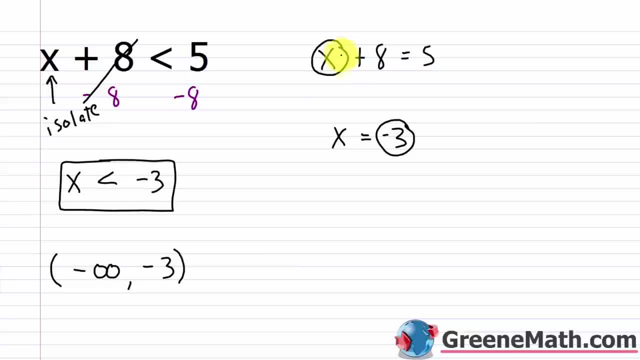 Okay. so I'm going to take this negative 3 and plug it in for x. So negative 3 plus 8 does equal 5, so that checks out. So this is right. here This is referred to as our boundary. Now the boundary is going to separate the solution region from the non-solution region. 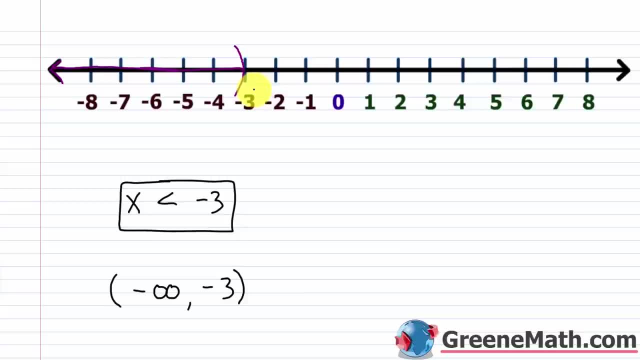 And graphically you can kind of see that negative 3 is the cutoff. Anything less than negative 3, anything over here works, So this is your solution region. Then anything starting at negative 3 and beyond doesn't work, So this is your non-solution region. 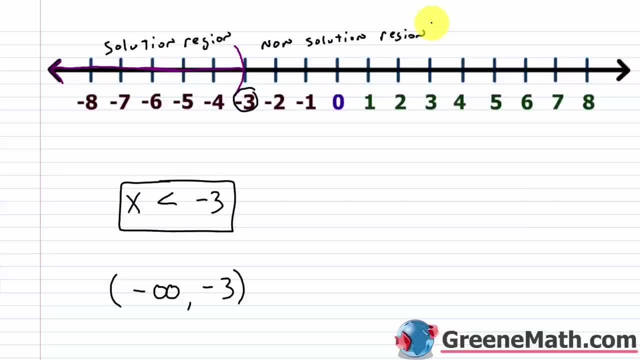 So what we need to do after we establish the boundary, we need to take a number from the non-solution region and try it, and then also a number from the solution region and try it. So, from the non-solution region, the easiest number to try is 0.. 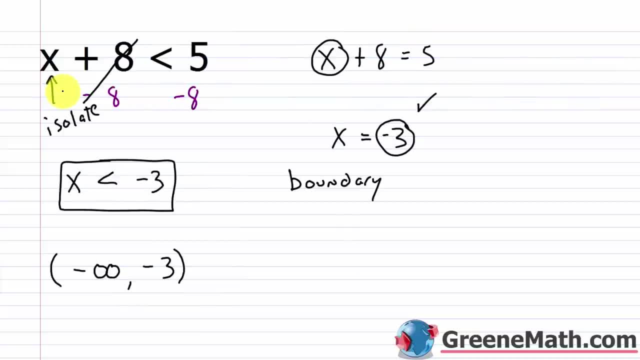 So let's go back up here and we can plug in a 0 for x and we'd have 8 is less than 5. So that's in the non-solution region. so it should be false and it is. 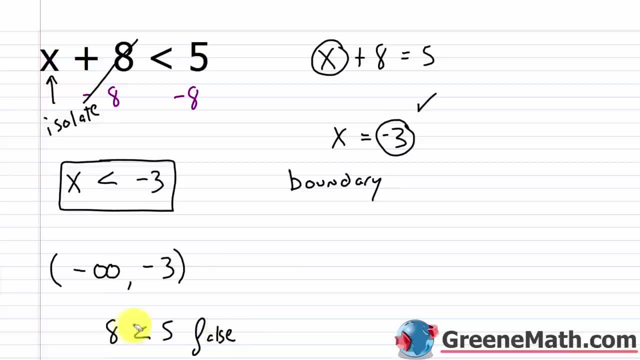 So it's okay that this is false. That's what we want. Now the next thing we're going to do is we're going to pick a number from the solution region. So that's over here. That's anything less than negative 3.. 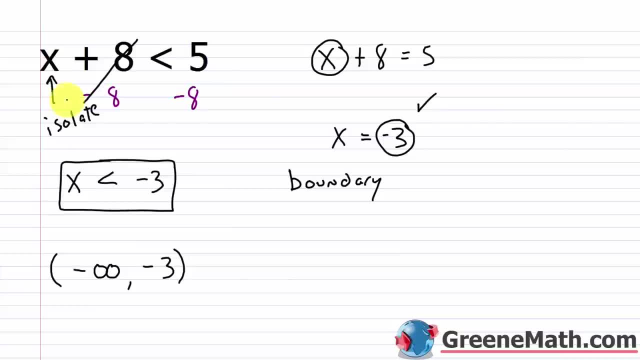 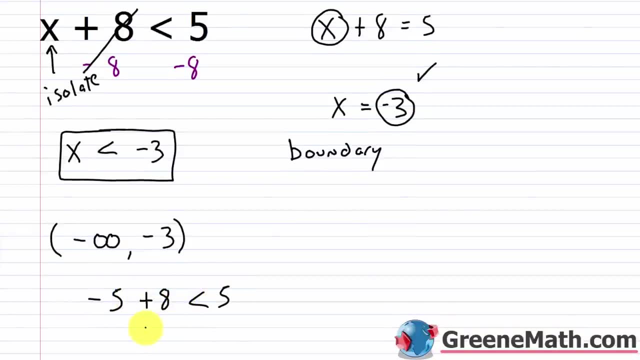 So I can pick anything I want. So let's say negative 5.. So I'd plug a negative 5 in for x. I'd have negative 5 plus 8 is less than 5.. Negative 5 plus 8 is 3, and 3 is less than 5.. 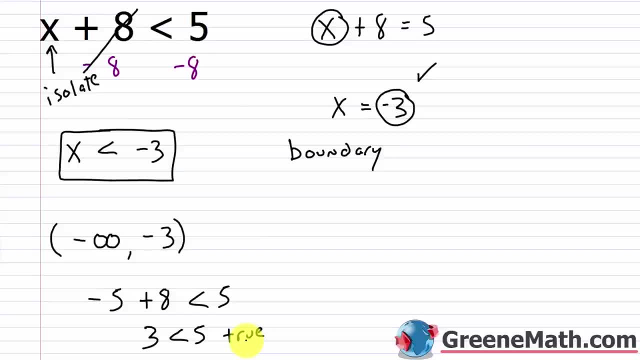 So that's true And that's exactly what we want, because we picked a number from the solution region. So again, a lot more complex to check your answer here, So I'm not going to do it moving forward, It's something that you can refer back to this procedure. 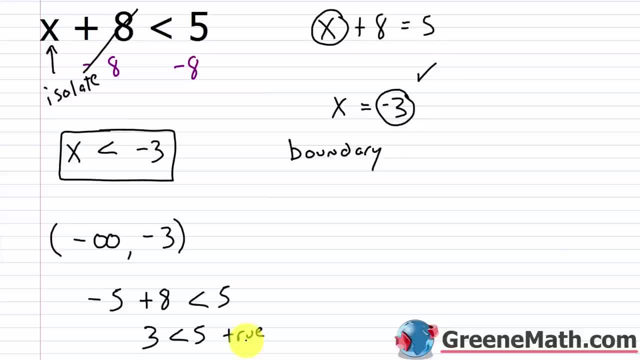 and you can check it on your own, because it is extremely time consuming. All right, let's take a look at the next one. So we have x plus 2 is less than or equal to 1.. So to solve this, I'm just going to subtract 2 away from both sides of the inequality. 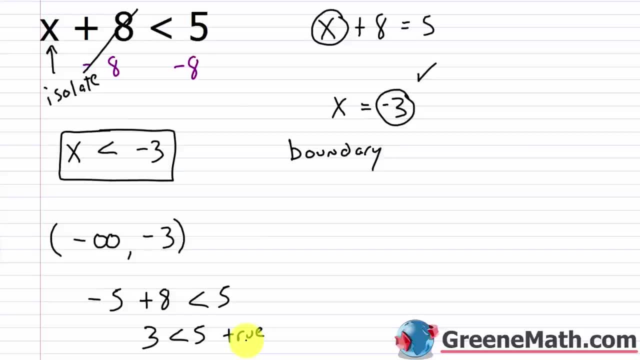 So that's true. And that's exactly what we want because we picked a number from the solution region. So again a lot more complex to check your answer here. So I'm not going to do it moving forward. It's something that you can refer back to this procedure and you can check it on your own 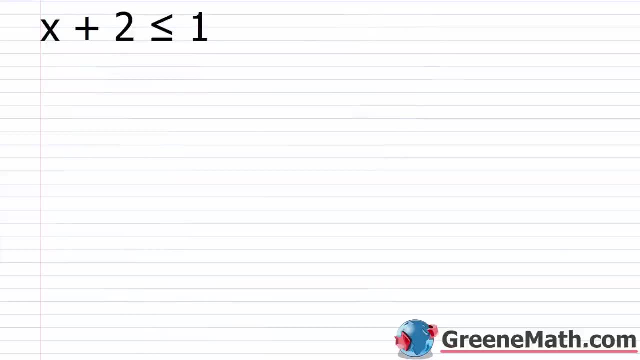 because it is extremely time consuming. Alright let's take 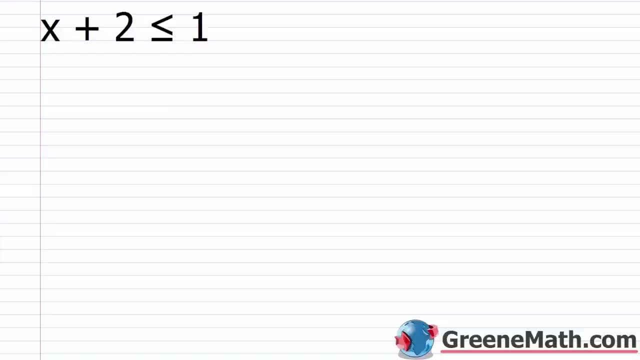 a look at the next one. So we have x plus 2 is less than or equal to 1. 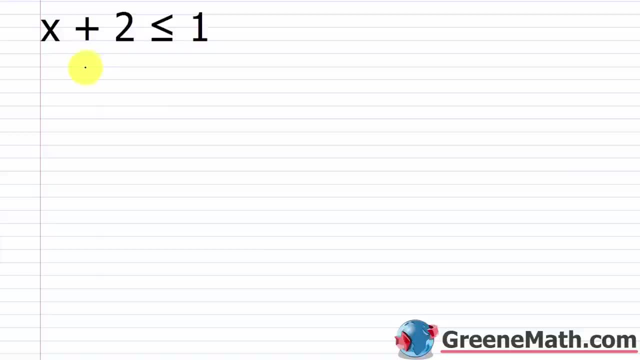 So to solve this I'm just going to subtract 2 away from both sides of the inequality. This will cancel. I'll have x by itself and I'll have less than or equal to 1 minus 2 is negative 1. So this is my solution. x is less than or equal to negative 1 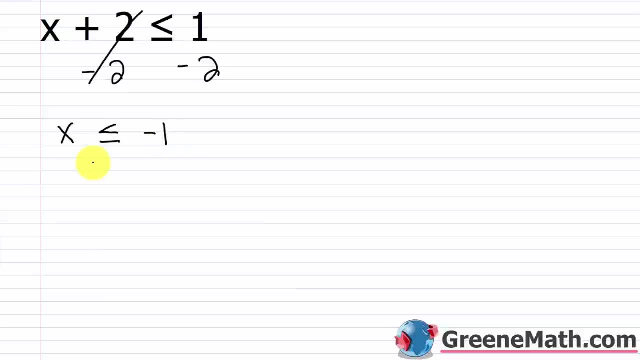 and to write this in interval notation again the smallest possible value we're dealing with a less than or equal to. So the smallest possible value is negative infinity because 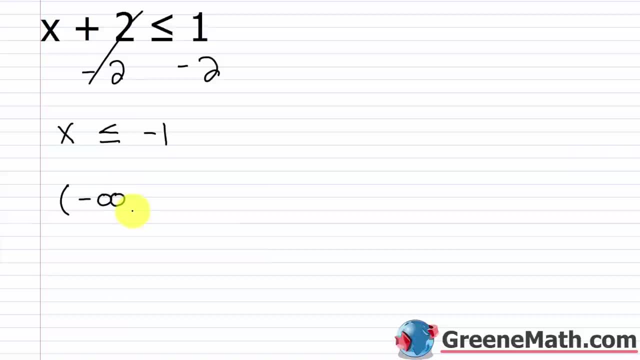 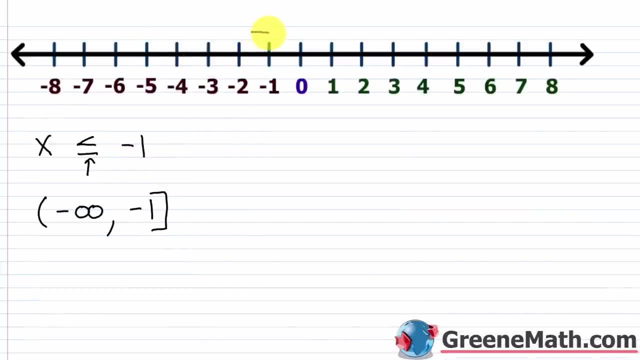 there is none. It continues forever and ever in the left direction. And then the largest possible value is negative 1. And because there's a non-strict inequality here negative 1 is included. So I'm going to use a bracket there. So graphically this is going to look like this. At negative 1 I'm going to put a bracket facing to the left and I'm going to shade everything to the left including that arrow. So this is x is less than or equal to negative 1. Alright let's take a look at 7x is less than 28. 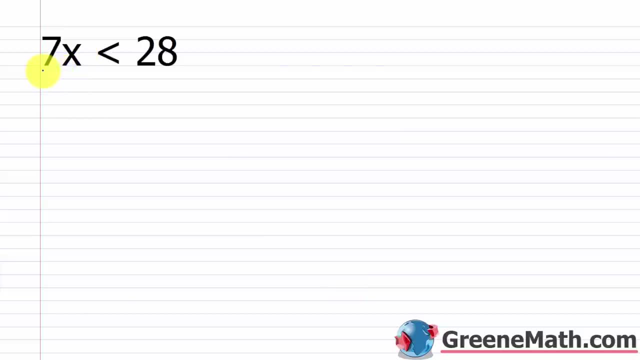 So if I want x by itself I need to divide both sides of the inequality by 7. Now remember I'm dividing by a positive number so I keep the direction of the inequality the same. This 7 cancels with this 7 and I'm just left with x and that is less than 28 divided by 7 is 4. 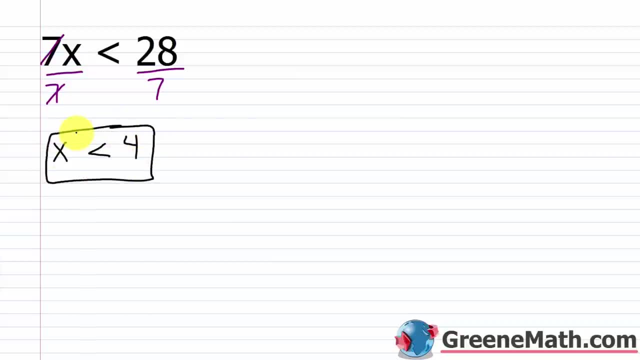 So that's my solution. x is less than 4. So in interval notation it's a less than so the smallest possible value is negative infinity because it continues forever and ever and ever in the left direction. Then the largest possible value, it's not quite 4 because 4 is not included but we're going to put 4 and then we're going to put a parenthesis next to that to say hey we can go all the way up to any amount that's close to 4 but we can't 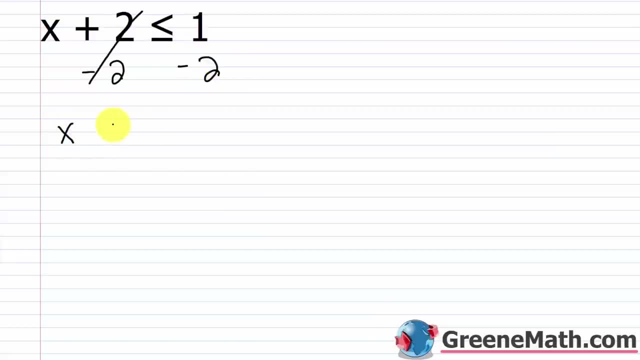 This will cancel. I'll have x by itself and I'll have less than or equal to 1 minus 2 is negative 1.. So this is my solution: x is less than or equal to negative 1.. And to write this in interval notation again: the smallest possible value. 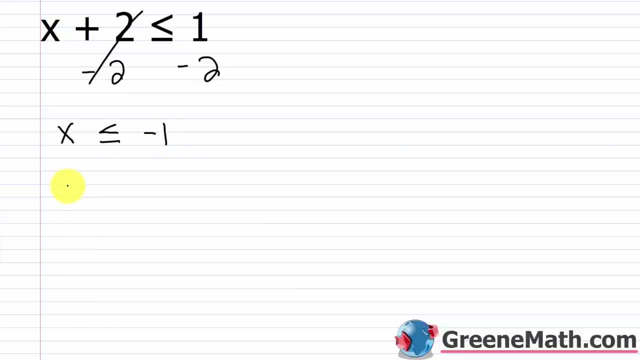 we're dealing with a less than or equal to, So the smallest possible value is negative, infinity right. because there is none, It continues forever and ever in the left direction. And then the largest possible value is negative, 1.. And because there's a non-strict inequality here, negative 1 is included. 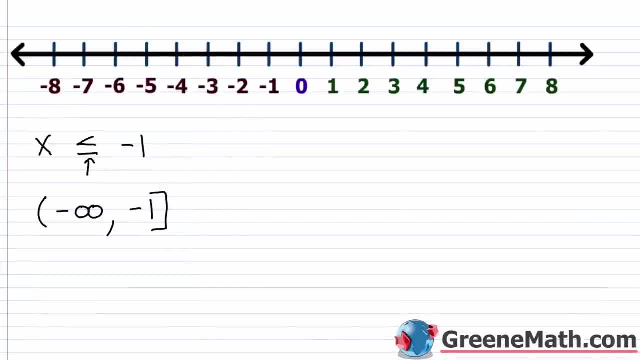 So I'm going to use a bracket there. So graphically this is going to look like this: At negative 1, I'm going to put a bracket facing to the left and I'm going to shade everything to the left, including that arrow. 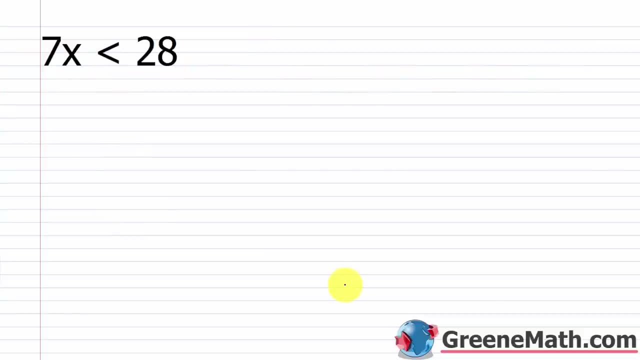 So this is: x is less than or equal to negative 1.. All right, let's take a look at 7x is less than 28.. So if I want x by itself, I need to divide both sides of the inequality by 7.. 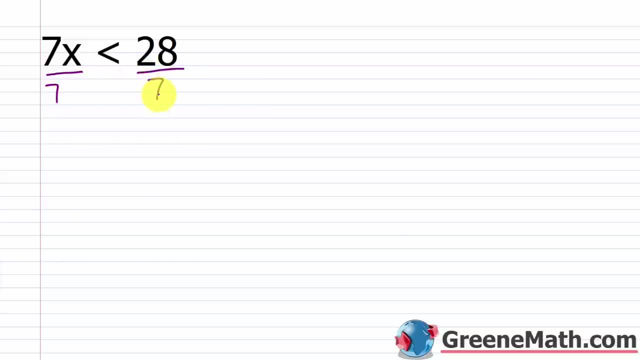 Now, remember, I'm dividing by a positive number, so I keep the direction of the inequality the same. This 7 cancels with this 7, and I'm just left with x, And that is less than 28 divided by 7 is 4.. 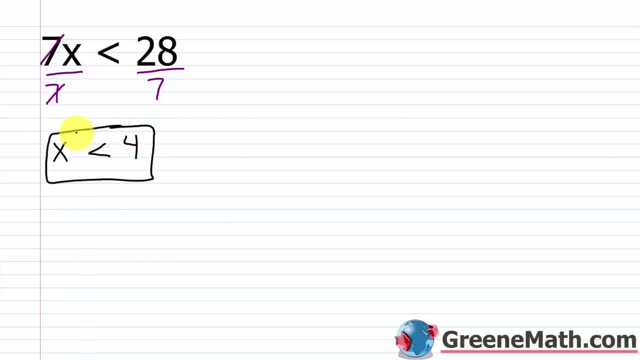 So that's my solution. x is less than 4. So in interval notation it's a less than So. the smallest possible value is negative infinity. right, because it continues forever and ever and ever in the left direction. Then the largest possible value is negative infinity. 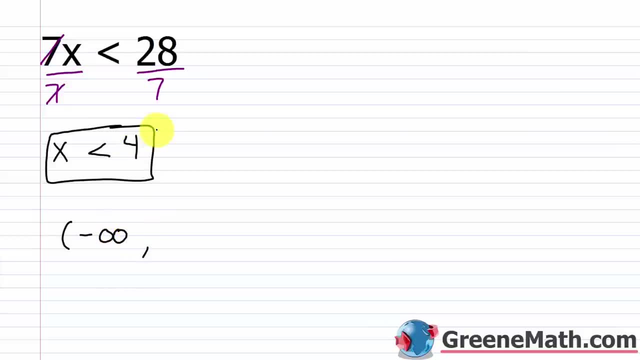 So the smallest possible value is negative infinity. It's not quite 4,, right, because 4 is not included, But we're going to put 4, and then we're going to put a parenthesis next to that to say, hey, we can go all the way up to any amount that's close to 4,. 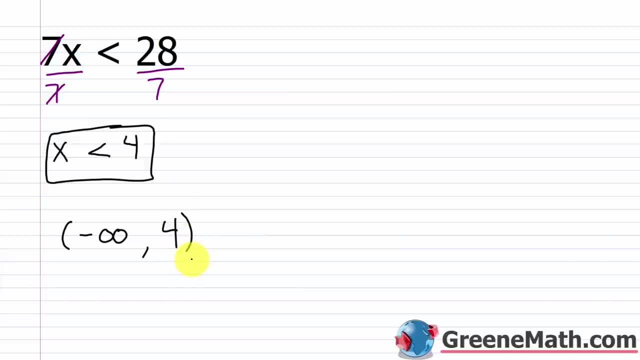 but we can't actually get to it. So again, this parenthesis is telling me that 4 is not included. Let me just make those even heights And let's graph x is less than 4.. All right, so I'd find 4 in the number line and that's right here. 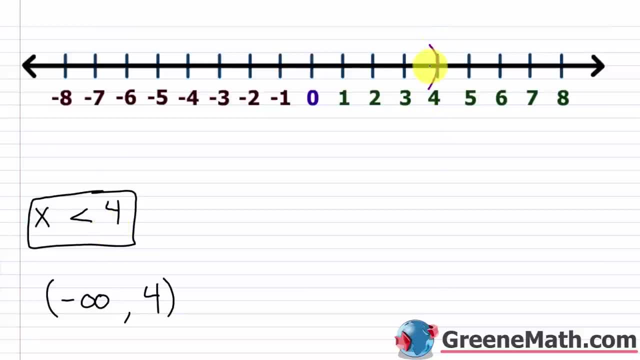 I'd put a parenthesis facing to the left, And then I'm going to shade everything to the left, Shade all this and shade the arrow to say, hey, x is less than 4.. So it can't quite be 4, but it can be anything less. 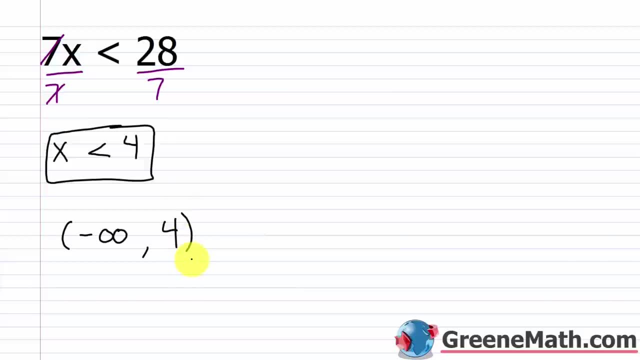 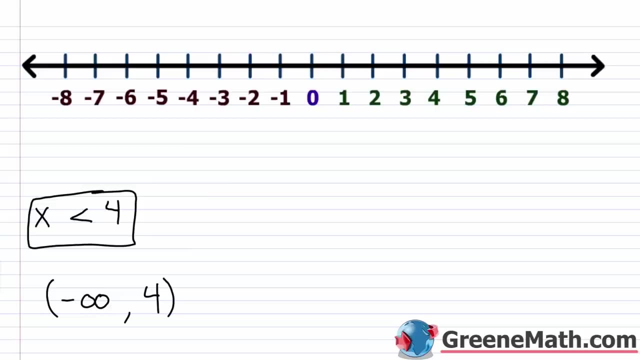 actually get to it. So again this parenthesis is telling me that 4 is not included. Let me just make those even heights and let's graph x is less than 4. Alright so I'd find 4 in the number line and that's right here. I'd put a parenthesis facing to the left and then I'm going to shade everything to the left. 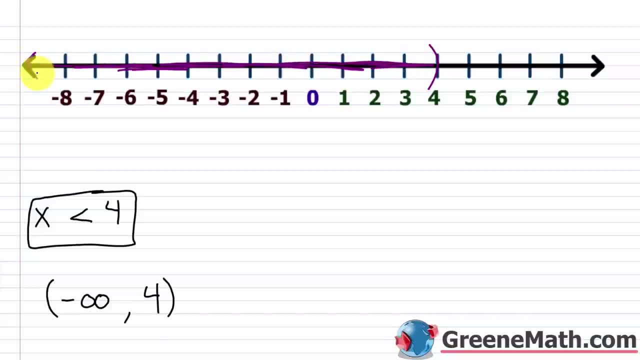 Shade all this and shade the arrow to say hey x is less than 4. So it can't quite be 4 but it can be anything less. 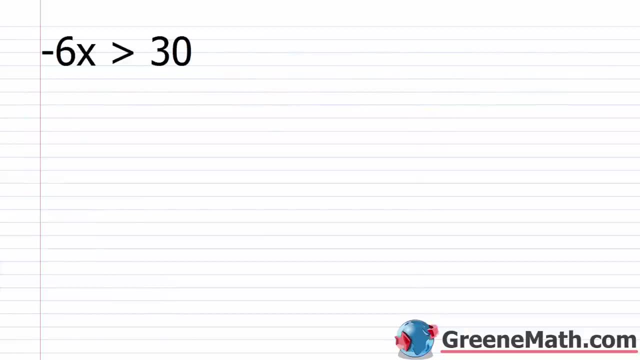 Alright let's take a look at negative 6x is greater than 30. 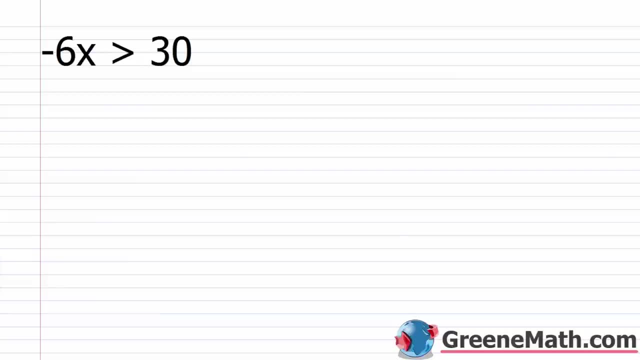 Now I want x by itself and in order to get x by itself I need to divide both sides of the inequality by the coefficient of x which is negative 6. 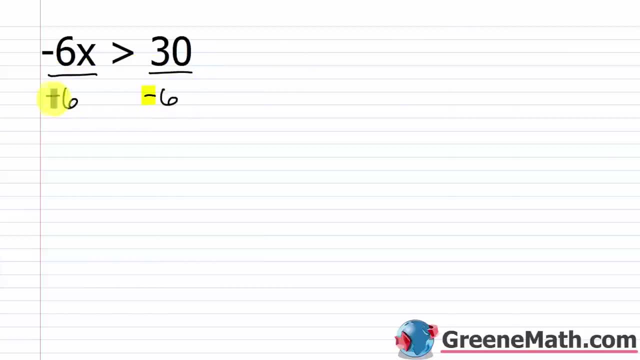 Now again I'm dividing by a negative. If I multiply or I divide by a negative I've got to flip the direction of the inequality. So do that first so you don't forget. So right now it's a greater than it needs to become a less than. So you flip it. Flip. Very important. 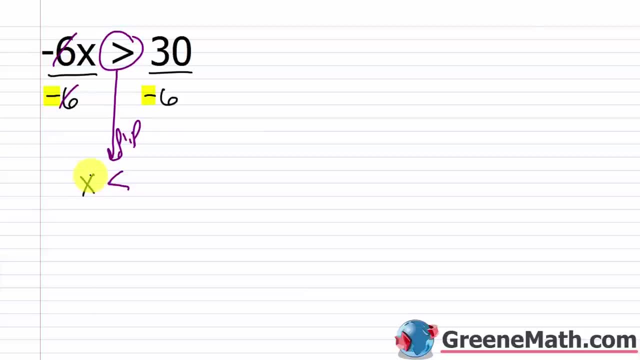 So this will cancel with this and I'll just have x and then 30 divided by negative 6 is negative 5. So x is less than negative 5. 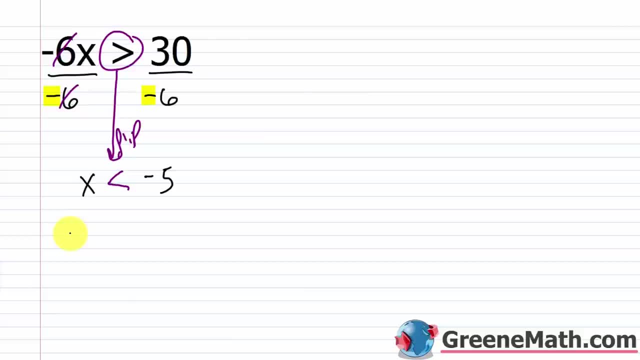 When we think about this in interval notation we know there's no possible way to get a smallest value. 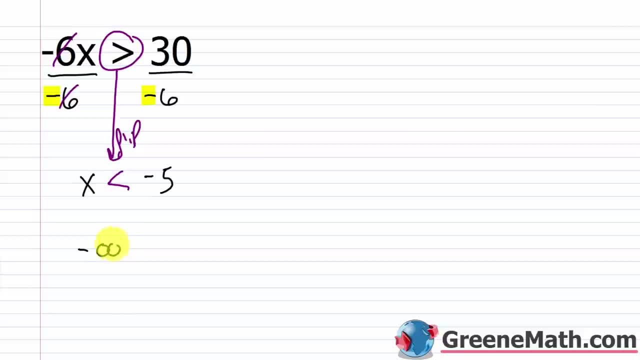 Alright so we're going to use negative infinity for that. Because the solution continues to go to the left forever. 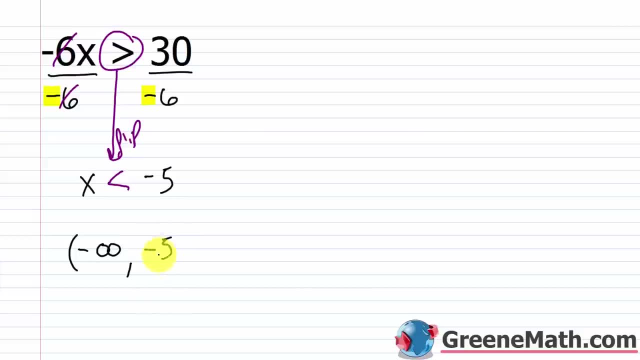 And then for the largest possible value I'm going to put negative 5 and then I'm going to put a parenthesis next to it to say hey negative 5 is not included. 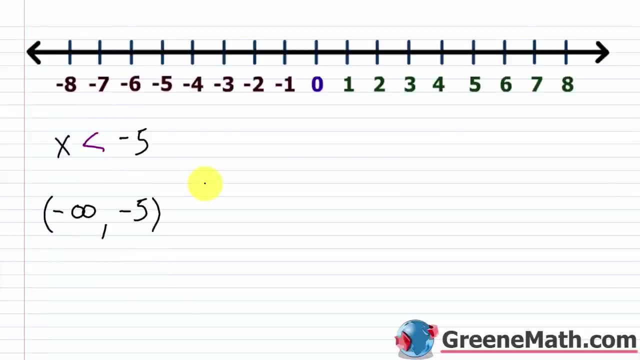 Now graphically when we look at this solution so I'm going to find negative 5 I'm going to put a parenthesis there and I'm going to shade everything to the left including that arrow to say hey negative 5 is not included 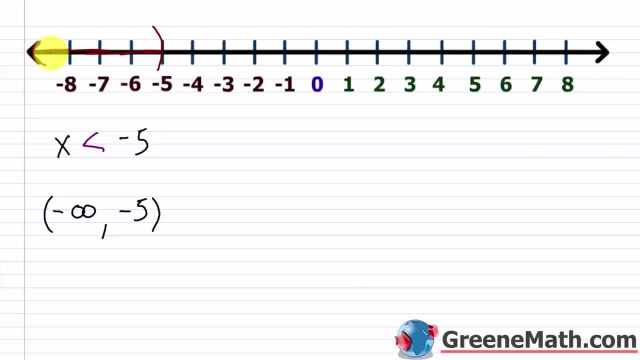 but everything to the left is and so x is less than negative 5 is the solution. 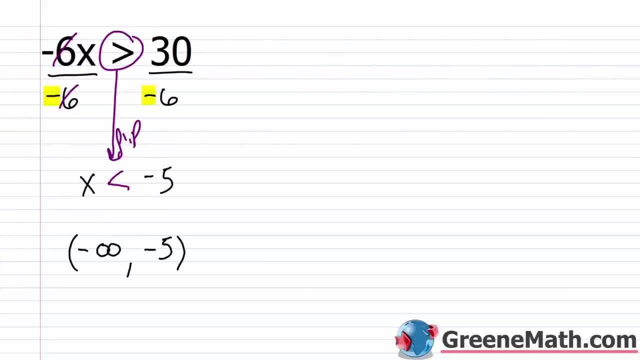 Now I know it's a little time consuming but I want to show you this very very important. 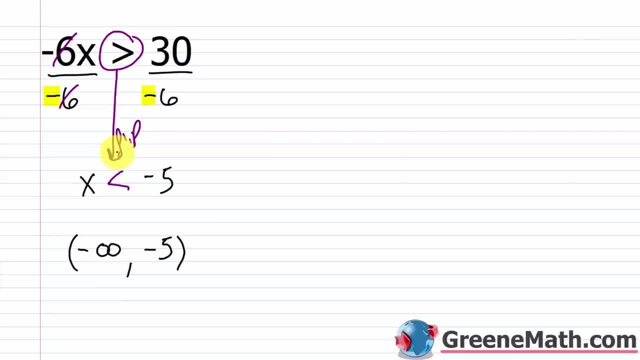 If I was to check this let's say that I did not flip the inequality. 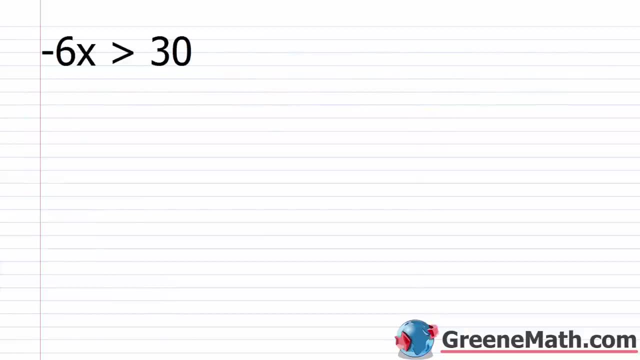 All right, let's take a look at negative 6x is greater than 30.. Now I want x by itself, And in order to get x by itself, I need to divide both sides of the inequality by the coefficient of x, which is negative 6.. 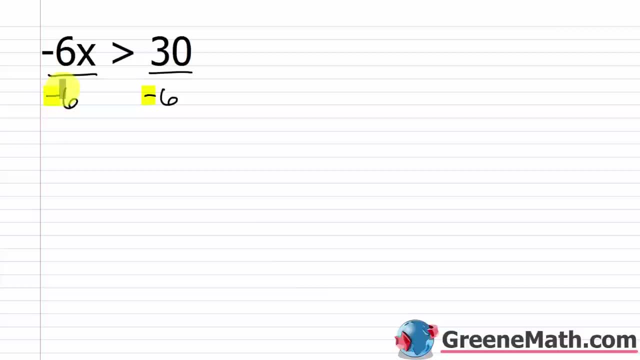 Now again, I'm dividing by a negative. If I multiply or I divide by a negative, I've got to flip the direction of the inequality. So do that first, so you don't forget. So right now it's a greater than. 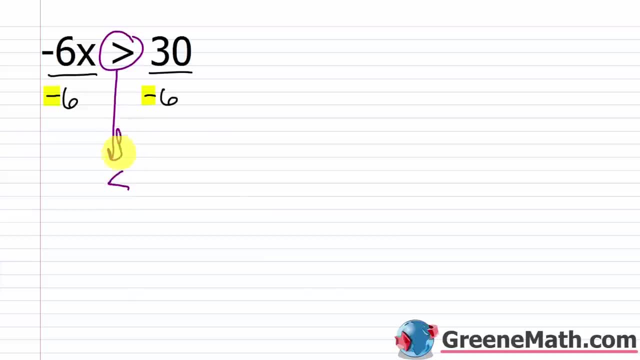 It needs to become a less than So you flip it. Flip Very important. So this will cancel with this And I'll just have x And then 30 divided by negative 6 is negative 5.. So x is less than negative 5.. 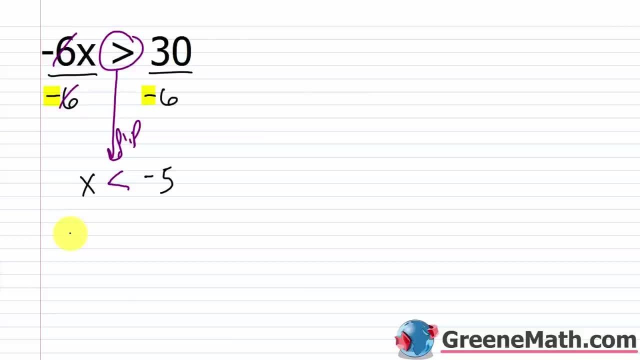 When we think about this in interval notation, we know there's no, There's no possible way to get a smallest value right. So we're going to use negative infinity for that, Because the solution continues to go to the left forever. And then for the largest possible value, I'm going to put negative 5.. 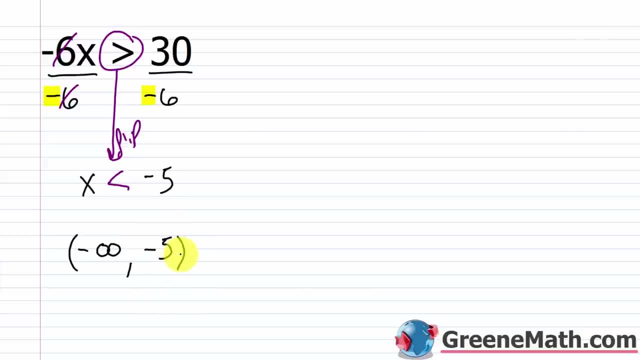 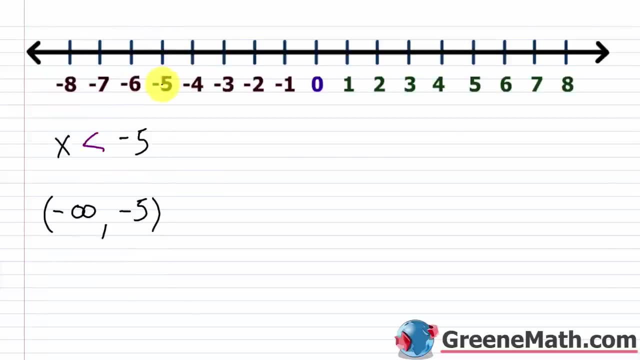 And then I'm going to put a parenthesis next to it to say, hey, negative 5 is not included Now, graphically, when we look at this solution. so I'm going to find negative 5.. I'm going to put a parenthesis there. 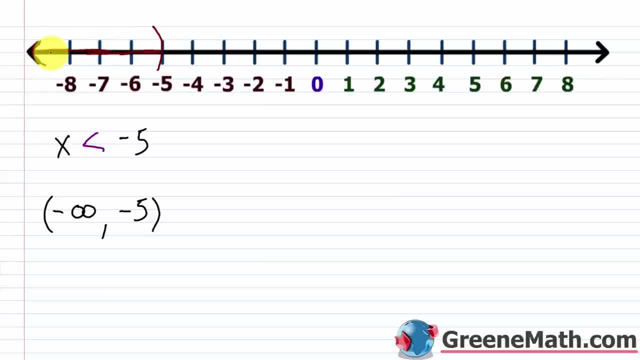 And I'm going to shade everything to the left, Including that arrow, to say, hey, negative 5 is not included, But everything to the left is, And so x is less than negative. 5 is the solution. Now, I know it's a little time consuming. 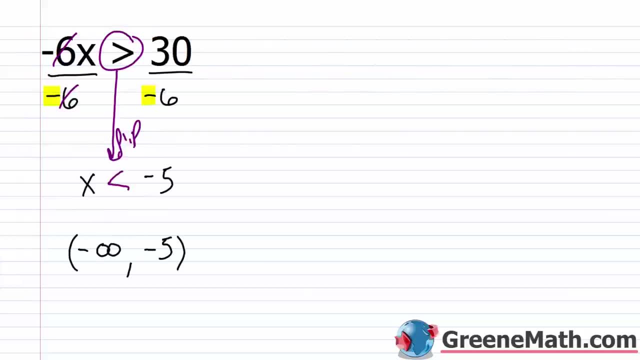 But I want to show you this Very, very important: If I was to check this, let's say that I did not flip the inequality. Let's say that I went through, I didn't flip this And I ended up with: x is greater than negative 5.. 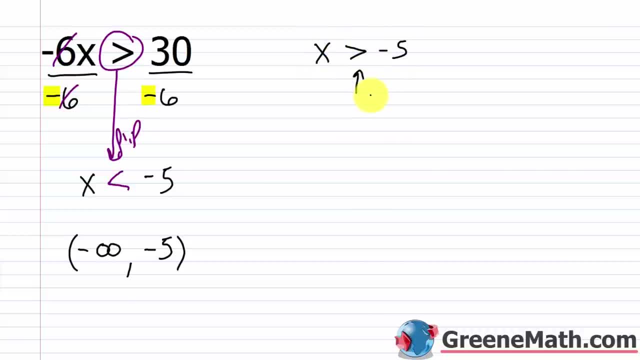 Let's say I said this is the solution. It's not. But I'm going to say I forgot to flip. All right, If you were checking this, the first thing you would do again is you would replace all your inequality symbols with equal symbols. 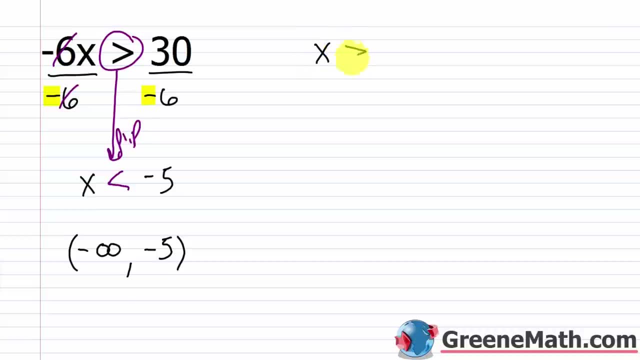 Let's say that I went through and I didn't flip this and I ended up with x is greater than negative 5. Let's say I said this is the solution. It's not but I'm going to say I forgot to flip. 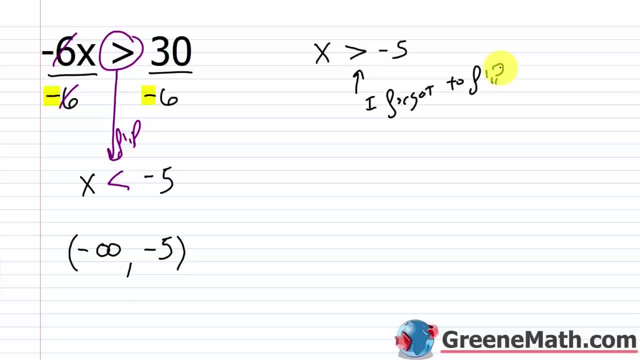 Alright. So we're checking this. 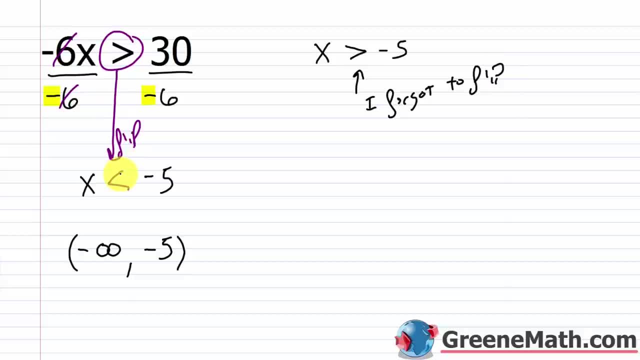 The first thing you would do again is you would replace all your inequality symbols with equal symbols. 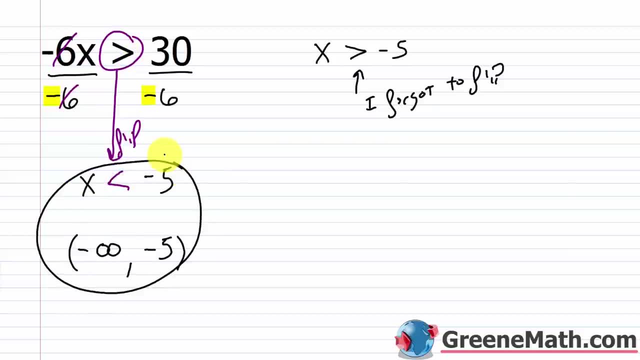 So in this case forget that this exists right now. This is gone. Just forget about it. 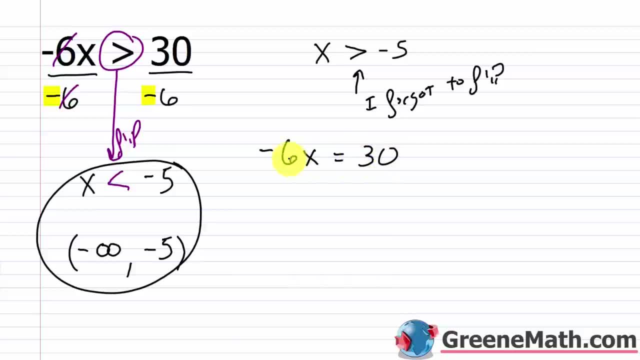 I would have negative 6x equals 30 as kind of the original thing. Then the solution is x equals negative 5. Okay. 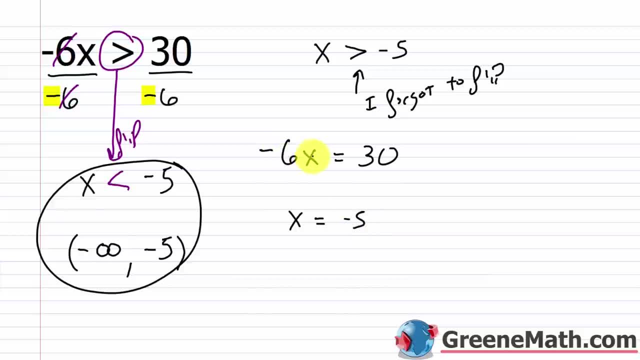 So if I plug a negative 5 into x I'd have negative 6 times negative 5 equals 30. So that works. 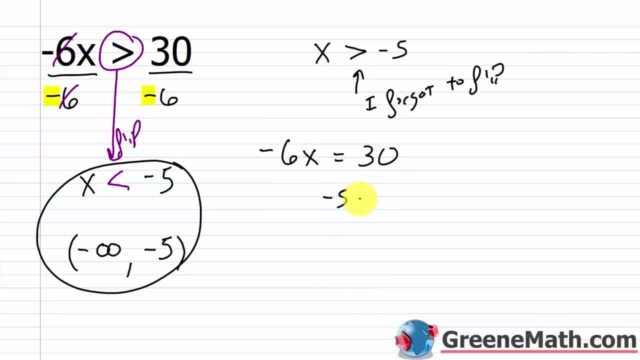 So I know that I have negative 5 as my boundary. 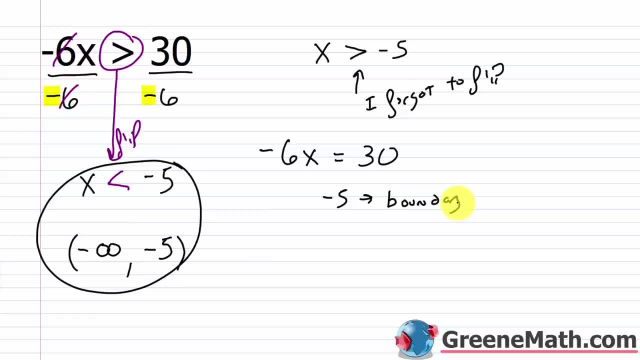 And again what that means is it separates the solution region from the non-solution region. 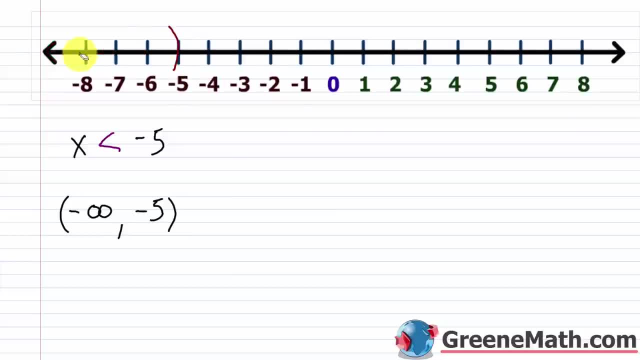 Graphically and again let me kind of erase this because we're kind of thinking about how to determine we have the wrong answer. 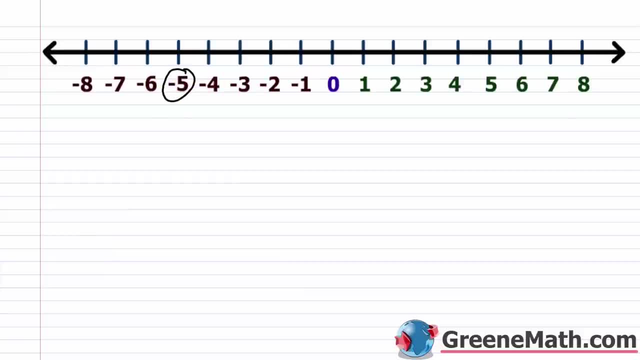 Graphically if I look at negative 5 if I came up with the wrong answer and I said x is greater than negative 5 I'd be thinking about okay anything larger than negative 5 would be in the solution region. 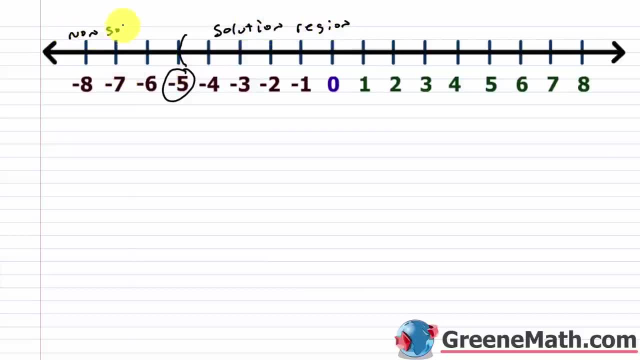 And anything less than negative 5 would be in the non-solution region. 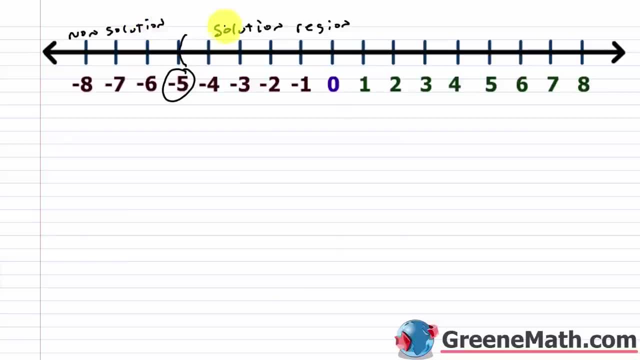 So if I tried something like 0 which should be in the solution region I'm going to find that I'm going to get the wrong answer. 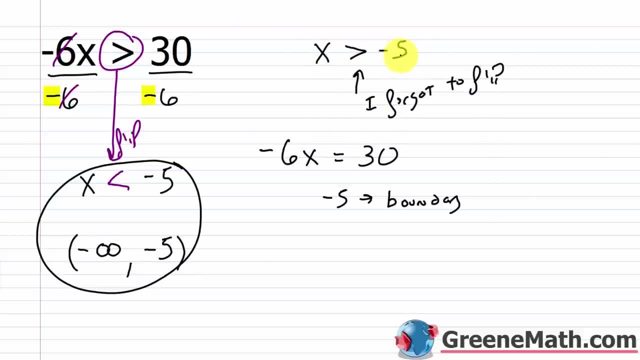 Because again I forgot to flip and 0 is greater than negative 5 so that works out here. 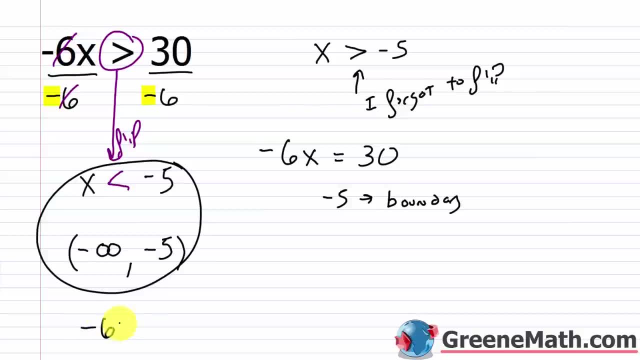 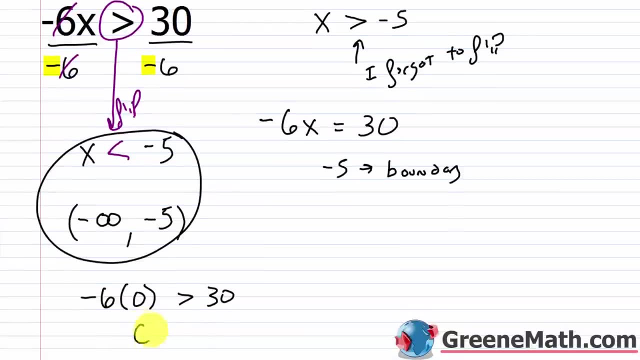 But in the original inequality which was negative 6 times x so I plug in a 0 there is greater than 30 well negative 6 times 0 is 0. That's not greater than 30. This would be false. 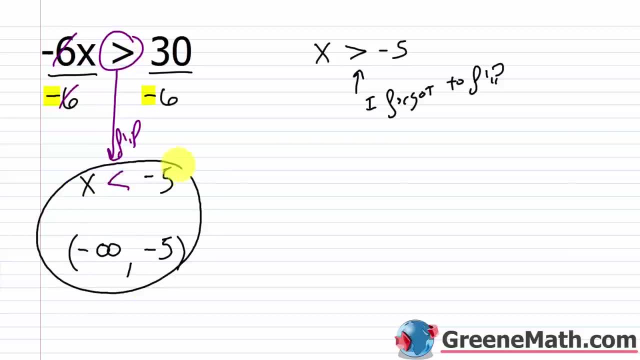 So in this case, forget that this exists right now. This is gone. Just forget about it. I would have negative 6x equals 30 as kind of the original thing. Then the solution is x equals negative 5.. Okay, So if I plug a negative 5 into x, I'd have negative 6 times negative 5 equals 30.. 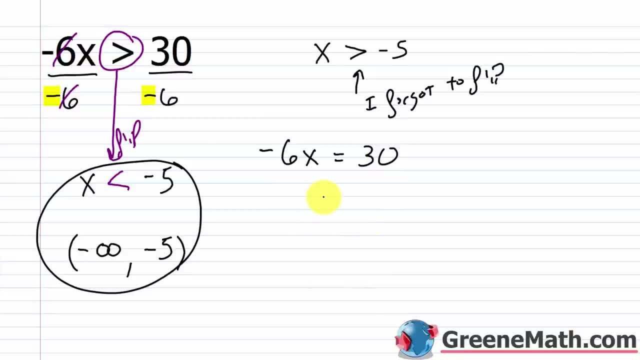 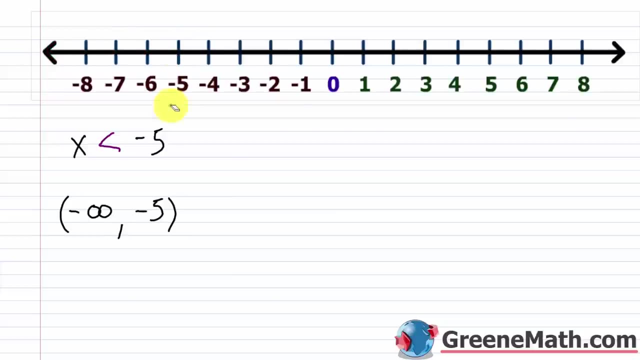 So that works. So I know that I have negative 5 as my boundary And again, what that means is it separates the solution region from the non-solution region Graphically. and again let me kind of erase this because we're kind of thinking about: 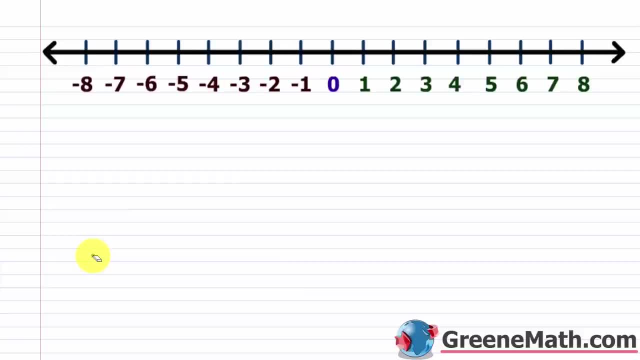 how to determine we have the wrong answer. Graphically, If I look at negative 5, if I came up with the wrong answer and I said x is greater than negative 5, I'd be thinking about: okay, anything larger than negative 5 would be in the solution region. 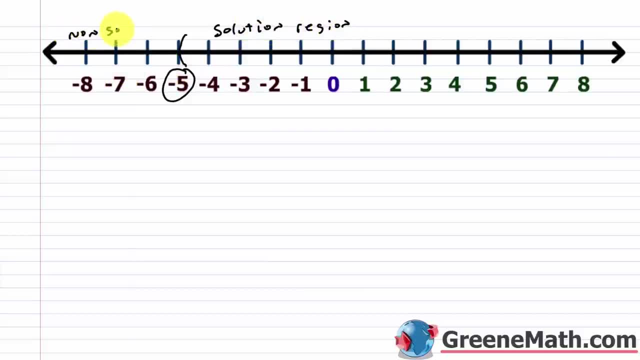 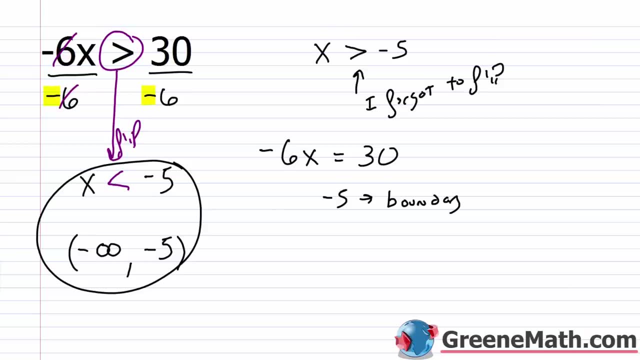 And anything less than negative 5 would be in the non-solution region. So if I tried something like 0,, which should be in the solution region, I'm going to find that I'm going to get the wrong answer Because again, I forgot to flip. 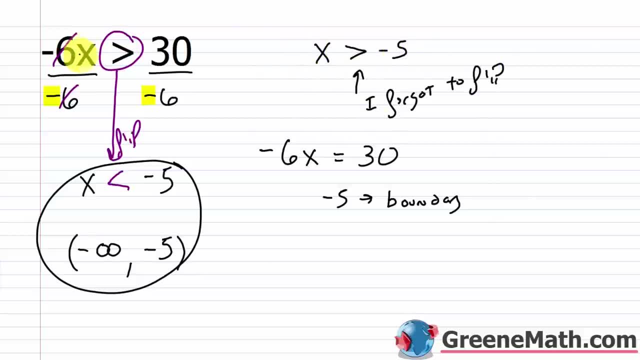 And 0 is greater than negative 5.. So that works out here. But in the original inequality, which was negative 6 times x- so I'd plug in a 0, there is greater than 30.. Well, negative 6 times 0 is 0.. 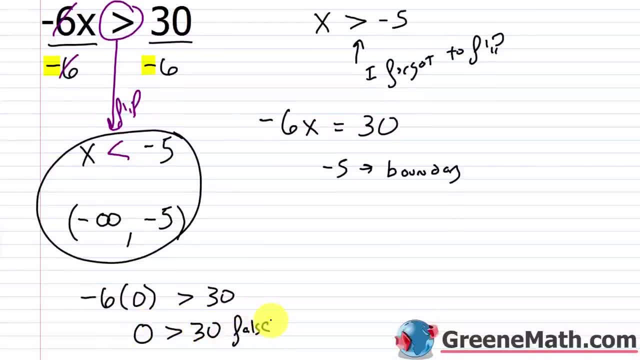 That's not greater than 30. This would be false. So that would be your first indication that something went wrong. I checked something that should have been in the solution region and it didn't work. Right. It did not work, So at that point I'd go up here and go: okay, this is false. 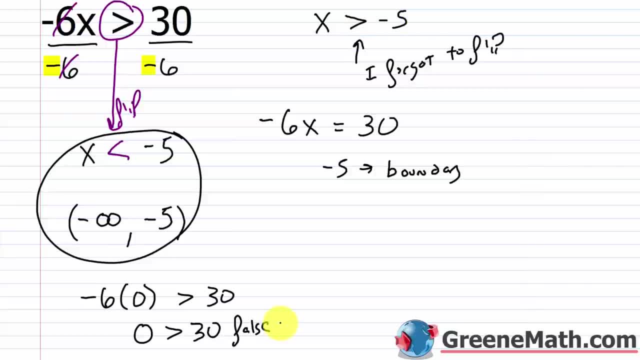 This doesn't work. This doesn't work. So I would go back And say, okay, well, I forgot to flip the inequality, So it's very time consuming to check, But when you first start doing these, you might want to just to avoid making the errors. 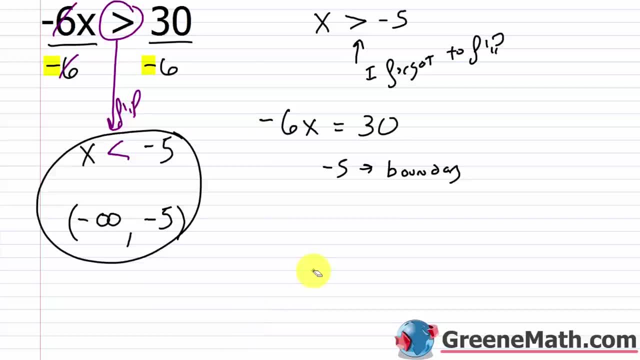 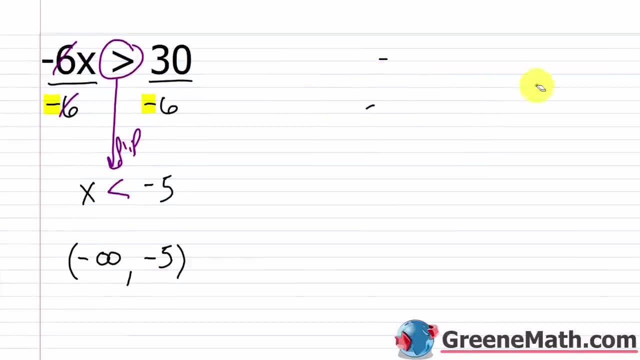 And let me show you what happens if you do this correctly. I know this is time consuming, but I feel like it's very important. So let's say I didn't forget to flip. We go back to our original solution. So x is less than negative 5.. 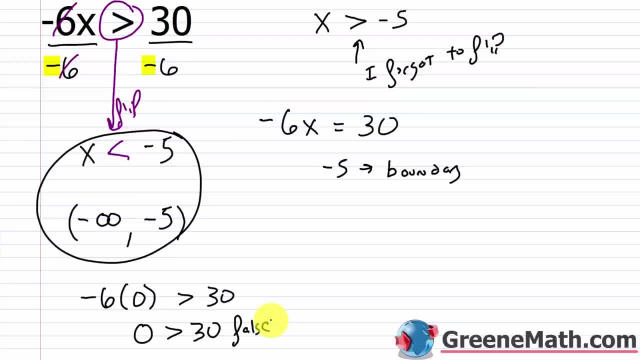 So that would be your first indication that something went wrong. I checked something that should have been in the solution region and it didn't work. It did not work. So at that point I'd go up here and go okay this is false. This doesn't work. This doesn't work. So I would go back and say okay well I forgot to flip the inequality. 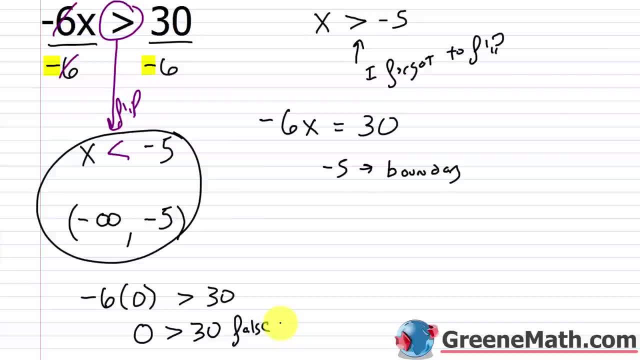 It's very time consuming to check but when you first start doing these you might want to just to avoid making the errors. 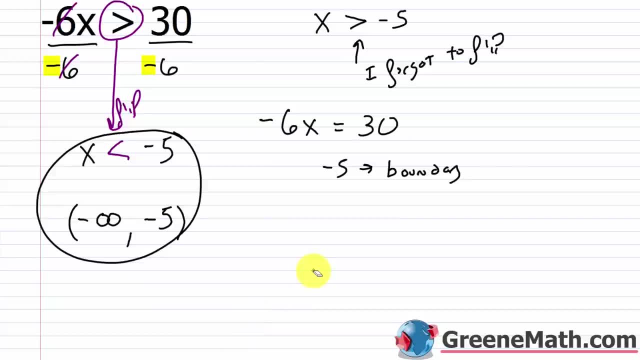 And let me show you what happens if you do this correctly. I know this is time consuming but I feel like it's very important. 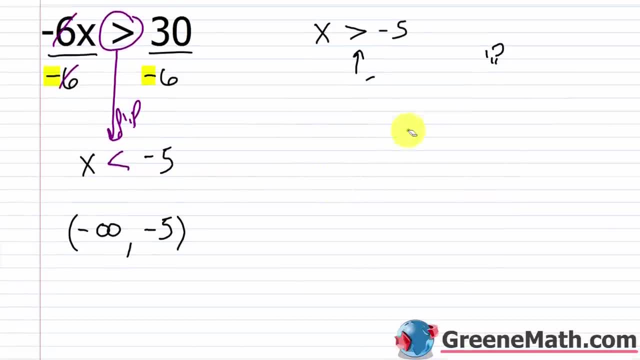 So let's say I didn't forget to flip. We go back to our original solution. 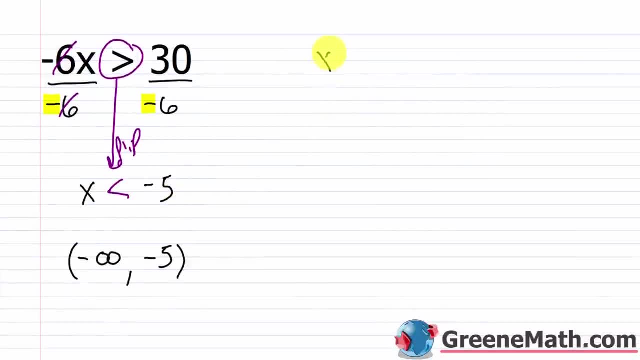 So x is less than negative 5 so we know our boundary is that x equals negative 5. So anything less than negative 5 should work as a solution. 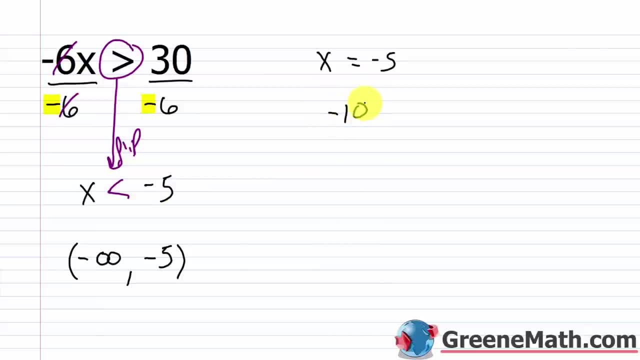 So if I plugged in a negative 10 for x that's less than negative 5 that would be in my solution region. 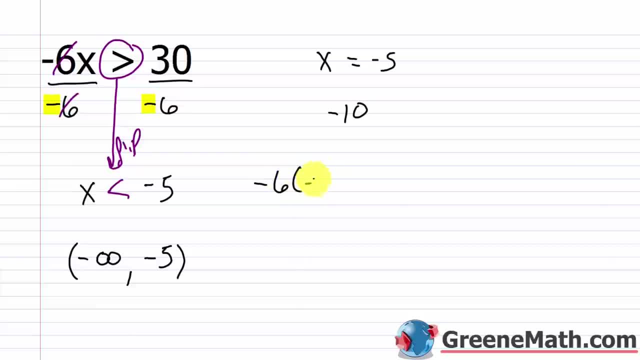 So it should give me a true result. So negative 6 times negative 10 should be greater than 30. Negative 6 times negative 10 is 60. That is greater than 30. That's true. 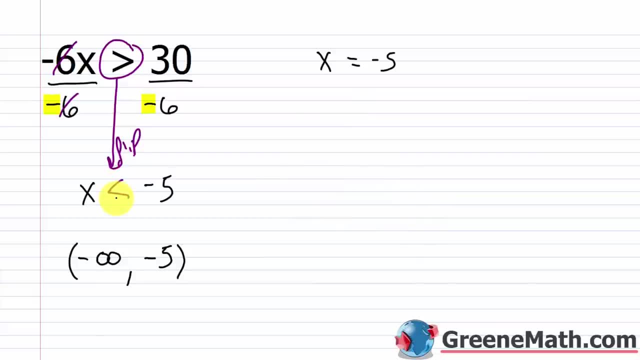 So that works out. That's exactly what we wanted. So if I use something like positive 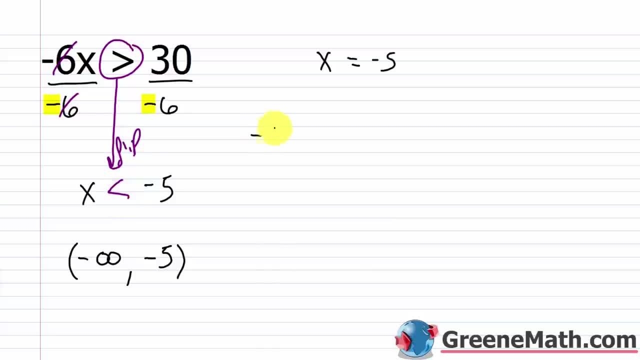 10 that should not be a solution. So I'd have negative 6 times 10 is greater than 30. 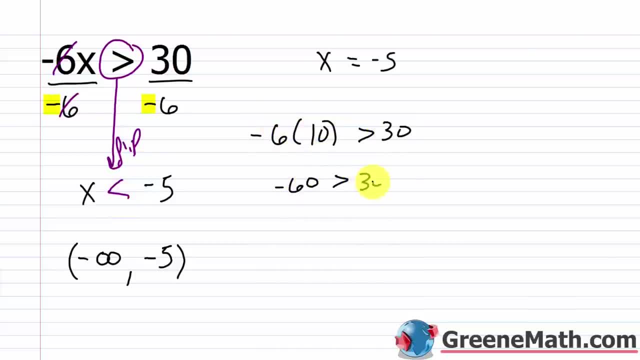 Negative 6 times 10 is negative 60. That's not greater than 30. That's false. So that's exactly what we want. That's okay. 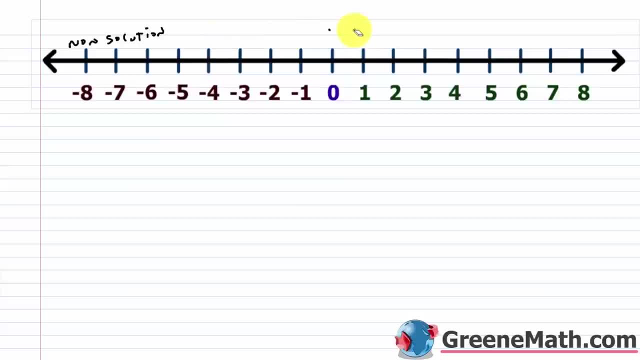 Again when you're checking this stuff and I have to reverse this because I gave you the scenario where we got the wrong answer. 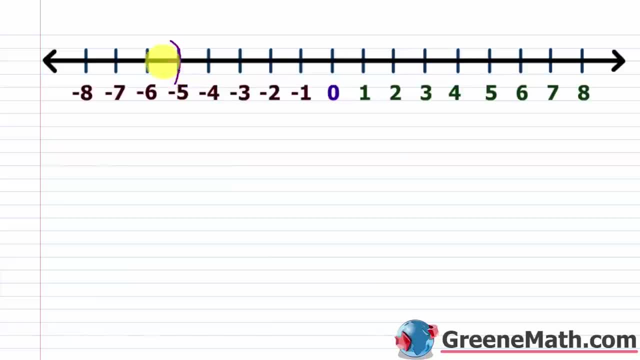 When you graph this anything less than negative 5 is in the solution region. 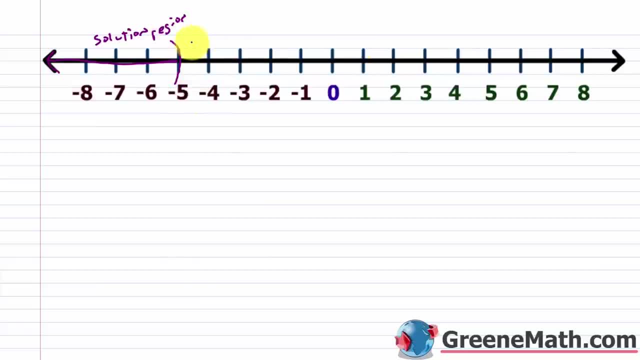 Anything that's negative 5 or larger is in the non-solution region. 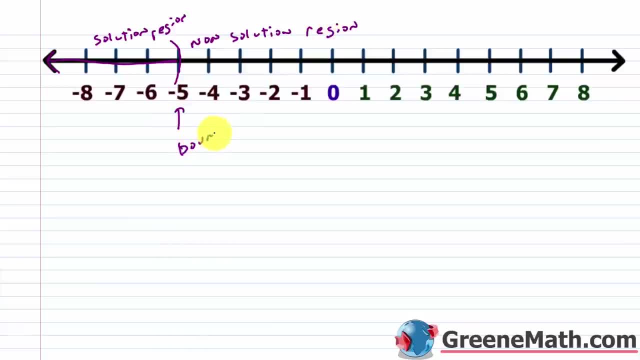 And again negative 5 is your boundary. It separates the 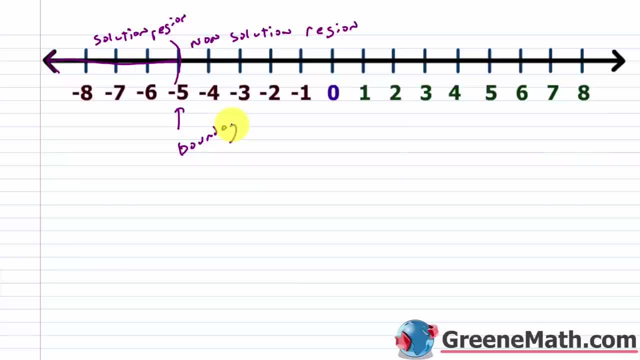 solution region from the non-solution region. And that's why you established that. 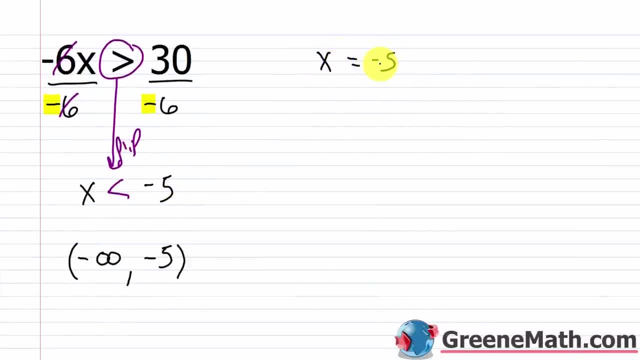 So we know our boundary is that x equals negative 5.. So anything less than negative 5. It should work as a solution, right? So if I plugged in a negative 10 for x, that's less than negative 5.. That would be in my solution region. 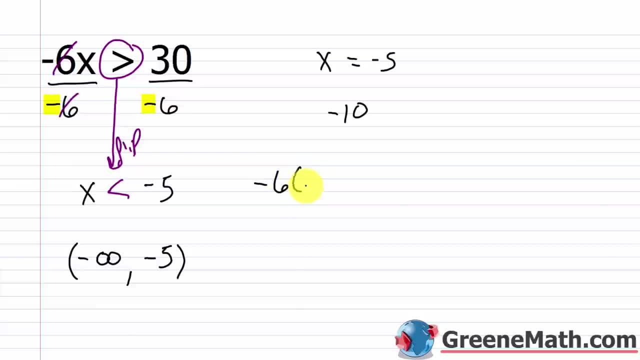 So it should give me a true result. So negative: 6 times negative: 10 should be greater than 30.. Negative: 6 times negative 10 is 60. That is greater than 30. That's true, So that works out. 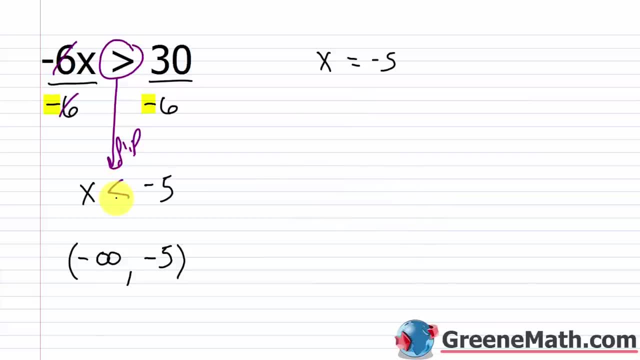 That's exactly what we wanted. So if I use something like positive 10, that should not be a solution. So I'd have: negative 6 times 10 is greater than 30.. Negative 6 times 10 is negative 60.. 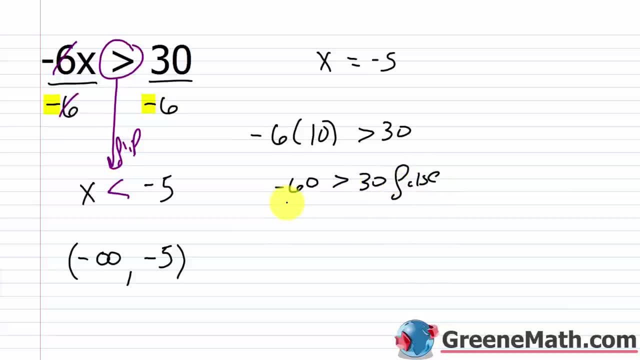 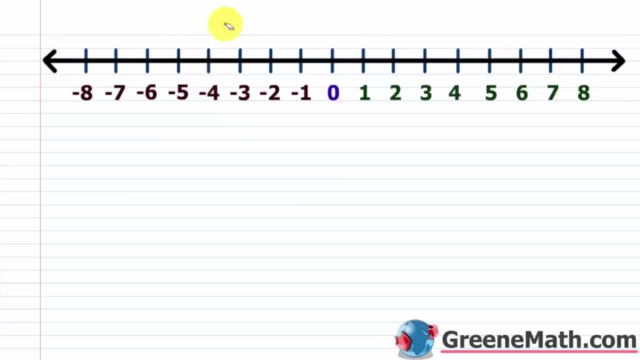 That's not greater than 30. That's false, right? So that's exactly what we want, That's okay, right? Again, when you're checking this stuff- and I have to reverse this because I gave you the scenario where we got the wrong answer- 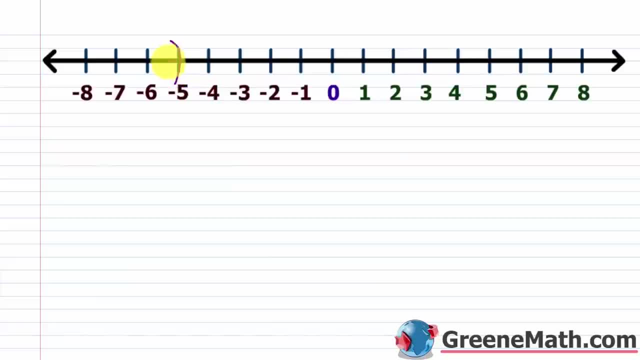 When you graph this, anything less than negative 5 is in the solution region. Anything that's negative 5 or larger is in the non-solution. So I'm going to take the solution region and I'm going to take the non-solution region. 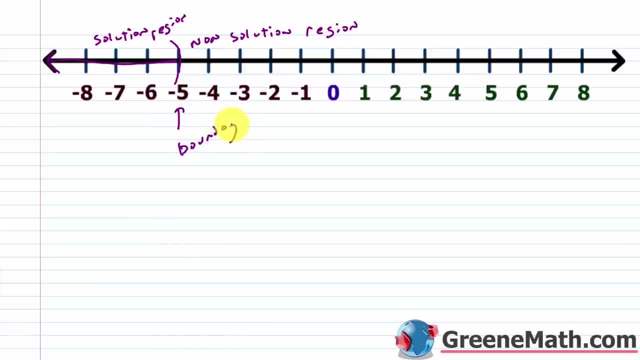 And again, negative 5 is your boundary. It separates the solution region from the non-solution region And that's why you establish that, So you can say: okay, I'm going to pick something on the non-solution and see if it works. 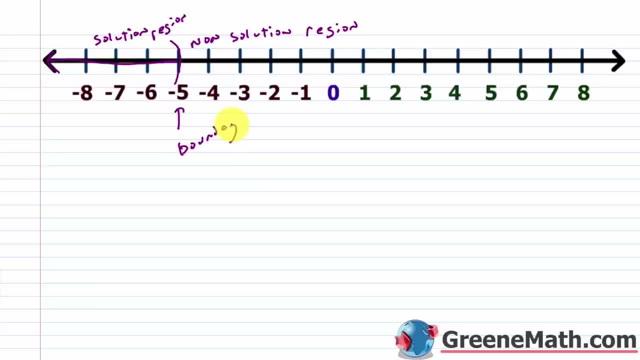 It shouldn't right because it shouldn't be a solution. And then I'm going to pick something on the solution region and that should work. And when we plugged in 10, 10 is in the non-solution region. It didn't work. 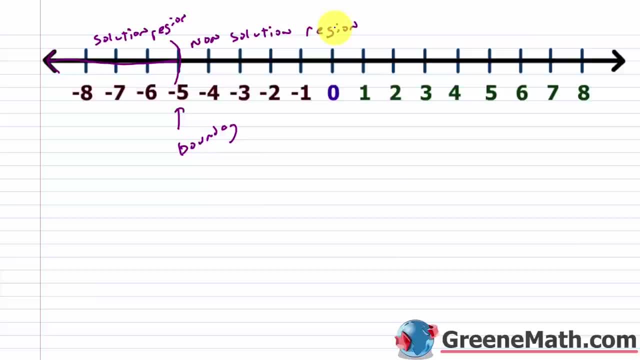 But when we took something from the solution region, we tried negative 10, it did work And that's what we want. All right, I know this video is kind of long, but when you first start out doing these, it's very important to get all the basics down. 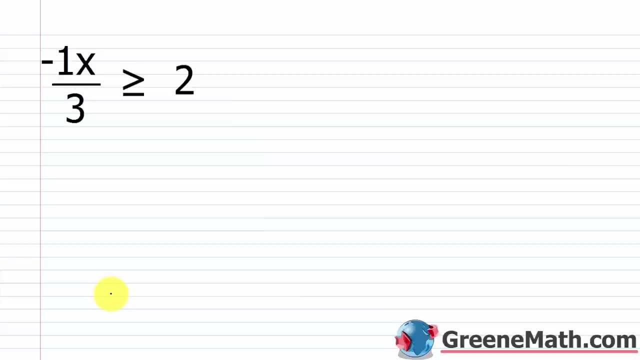 So it's kind of worth the time, even if you have to break it up. So we're going to look at one final problem. here We have negative 1 third x is greater than or equal to 2.. So if I want to isolate x and I have a fractional coefficient, I have a fractional coefficient. 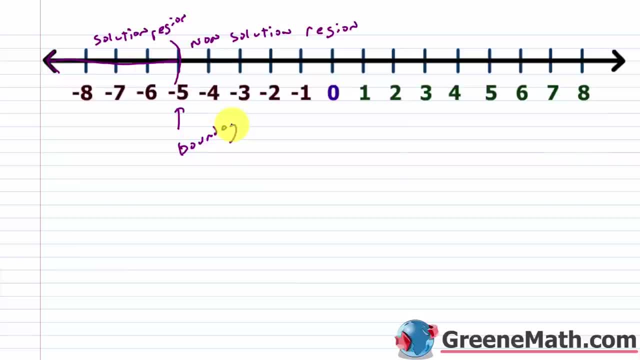 So you can say okay I'm going to pick something on the non-solution and see if it works. It shouldn't because it shouldn't be a solution. And then I'm going to pick something on the solution region and that should work. And when we plugged in 10, 10 is in the non-solution region, it didn't work. That's what we want. When we plugged in something from the solution region, we tried negative 10 it did work. And that's what we want. 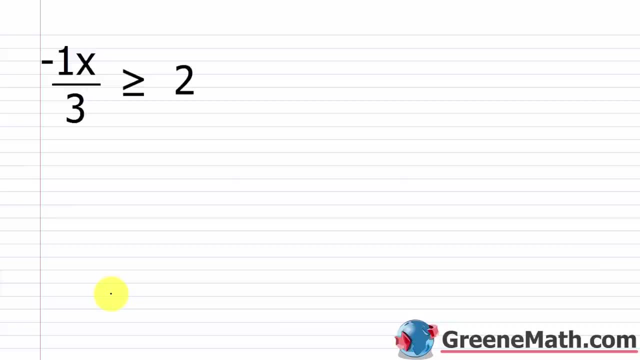 Alright I know this video is kind of long but when you first start out doing these it's very important to get all the basics down. So it's kind of worth the time. Even if you have to break it up. 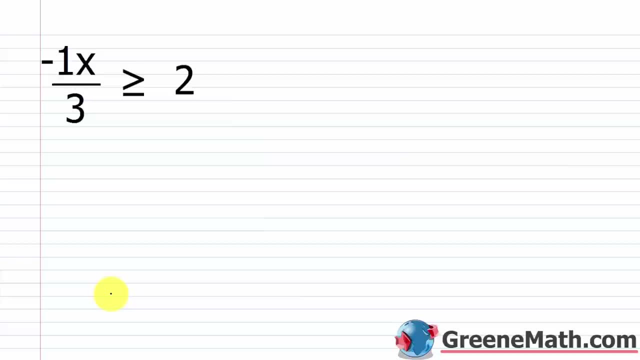 So we're going to look at one final problem here. We have negative 1 third x is greater than or equal to 2. So if I want to isolate x and I have a 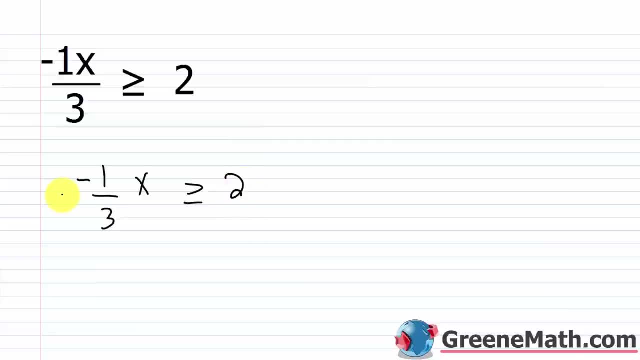 I have a fractional coefficient. We know what to do. We multiply both sides of the inequality by the reciprocal. So the reciprocal of negative 1 third is negative 3 over 1. And remember we're multiplying by a negative. So we've got to flip this. 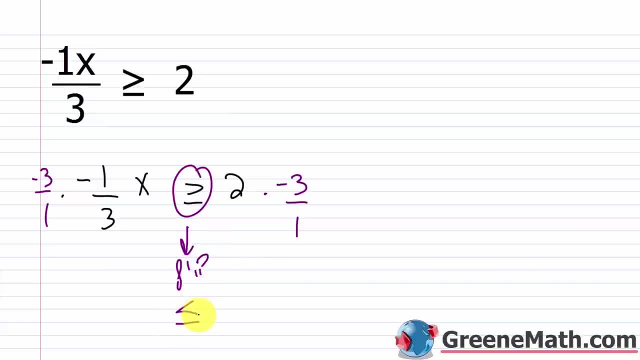 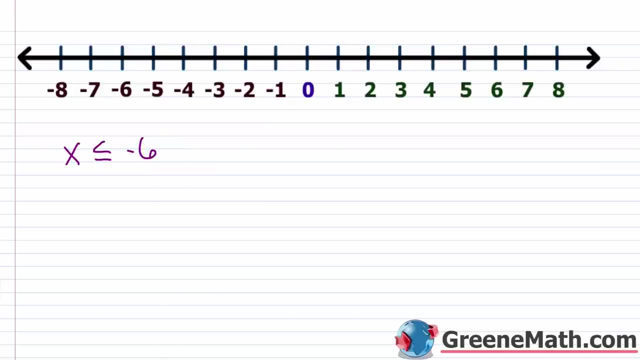 So this is going to go this way. So instead of greater than or equal to it's now less than or equal to. This is going to cancel and I'm just going to have x is less than or equal to 2 times negative 3 is negative 6. So x is less than or equal to negative 6. Let's do the interval notation for that. 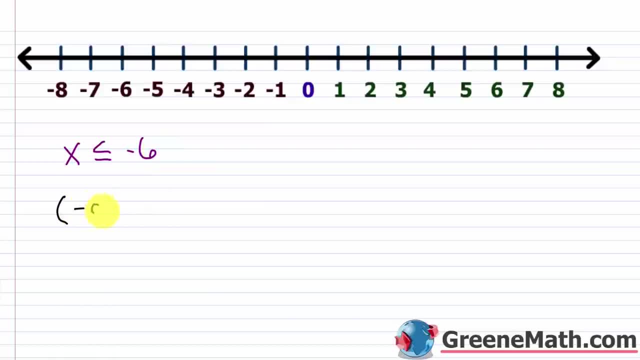 So it's going to be negative infinity over here on the left. 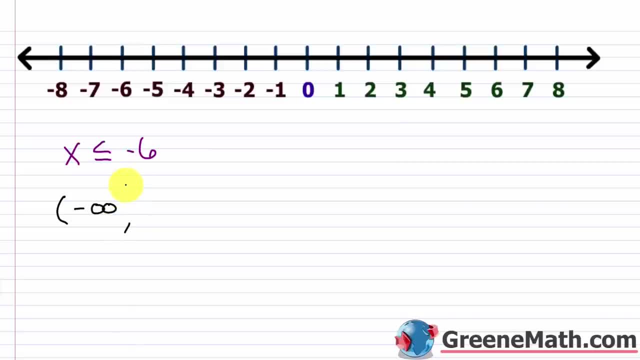 Because we're not going to have a smallest possible value. So we use negative infinity. 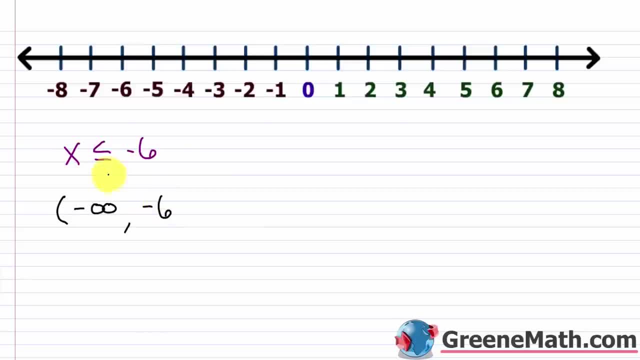 And then for the largest possible value we're going to use negative 6. And that's included because this is a non-strict inequality. So we're going to use a bracket next to negative 6. 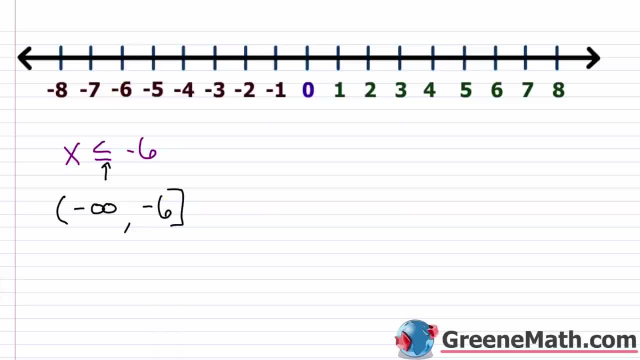 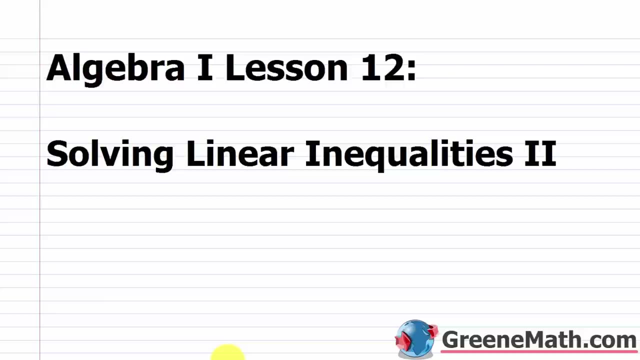 Now graphically I'm going to find negative 6 and I'm going to put a bracket there facing to the left. And I'm going to shade everything to the left. And I'm saying hey, negative 6 is a solution. That's why I've got the bracket. Anything to the left is also a solution. Hello and welcome to Algebra 1 Lesson 12. 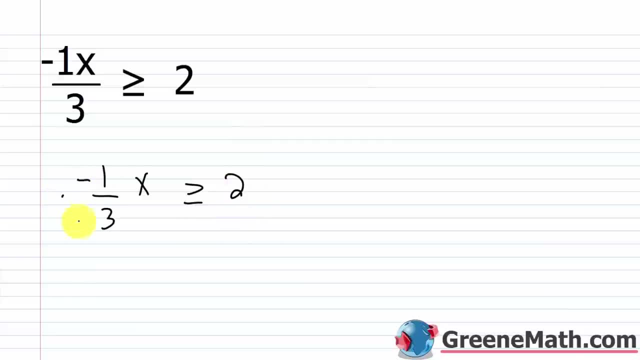 I'm going to multiply both sides of the inequality by the reciprocal. So the reciprocal of negative 1 third is negative 3 over 1.. And remember we're multiplying by a negative, So we've got to flip this. So this is going to go this way. 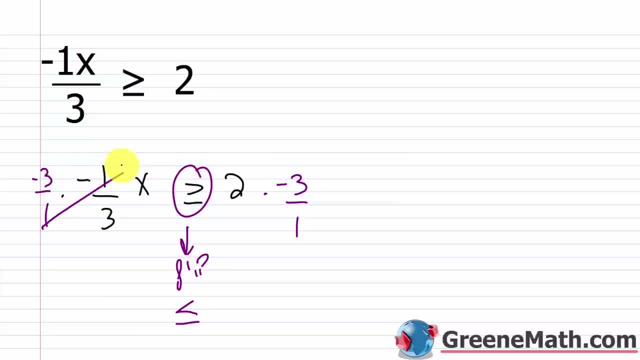 So, instead of greater than or equal to, it's now less than or equal to. This is going to cancel and I'm just going to have: x is less than or equal to 2 times negative. 3 is negative 6.. x is less than or equal to negative 6.. 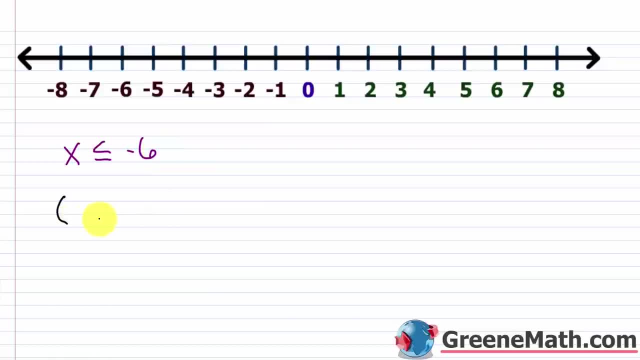 Let's do the interval notation for that. So it's going to be negative infinity over here on the left right, Because we're not going to have a smallest possible value. So we use negative infinity And then for the largest possible value we're going to use negative 6.. 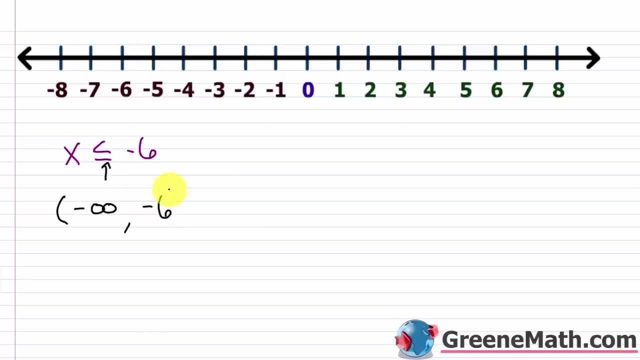 And that's included, because this is a non-strict inequality. So we're going to use a bracket next to negative 6.. Now, graphically, I'm going to find negative 6 and I'm going to put a bracket there Facing to the left. 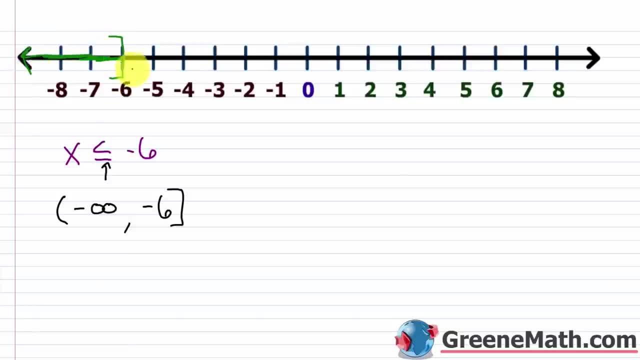 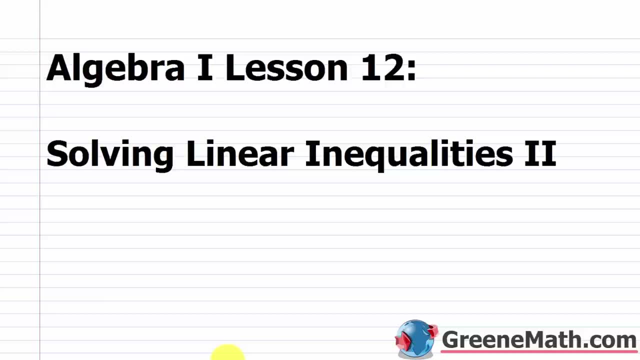 And I'm going to shade everything to the left And I'm saying, hey, negative 6 is a solution. That's why I got the bracket. And then anything to the left is also a solution. Hello and welcome to Algebra 1, Lesson 12.. 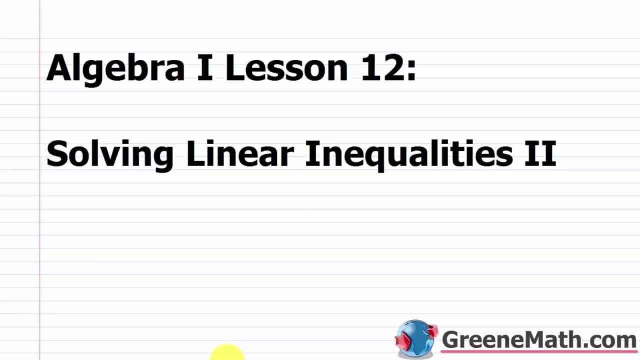 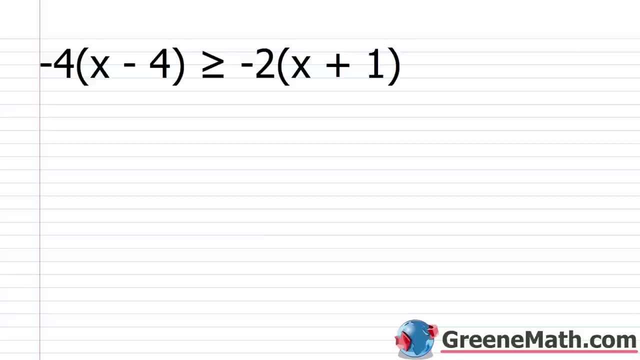 In this video we're going to continue learning about how to solve linear inequalities in one variable. So we're just going to kind of jump in here. We already know the basics, And so anything else that we're going to learn we're going to learn along the way. 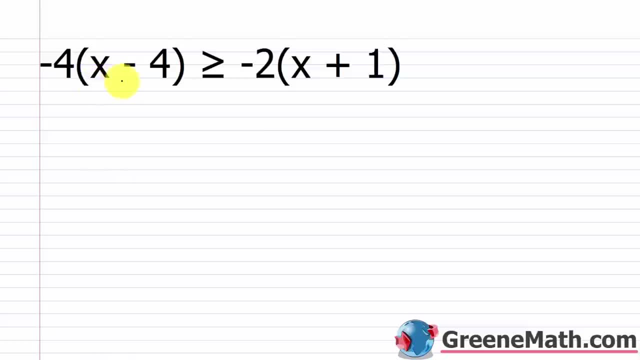 So when I look at this, I have negative 4 times the quantity x minus 4, is greater than or equal to negative 2 times the quantity x plus 1.. Now, the same way I would do an equation, I'm going to simplify each side completely. 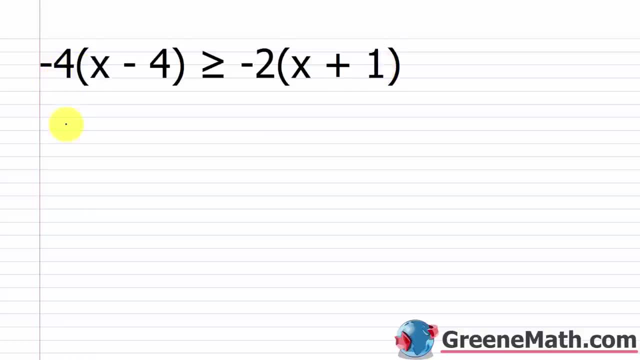 So I'm going to use my distributive property on the left. Negative 4 times x is negative 4x. Then I have negative 4 times negative 4. That's plus 16. And this is greater than or equal to. 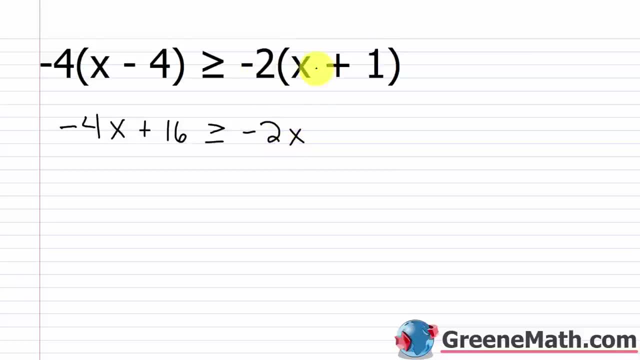 We have negative 2 times x, That's negative 2x, And then negative 2 times 1. That's minus 2.. Now, just like with an equation, I want all my variable terms on one side of the inequality and all my numbers on the other. 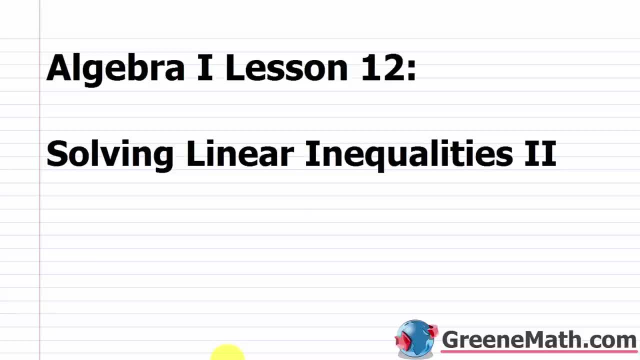 In this video we're going to continue learning about how to solve linear inequalities in one variable. 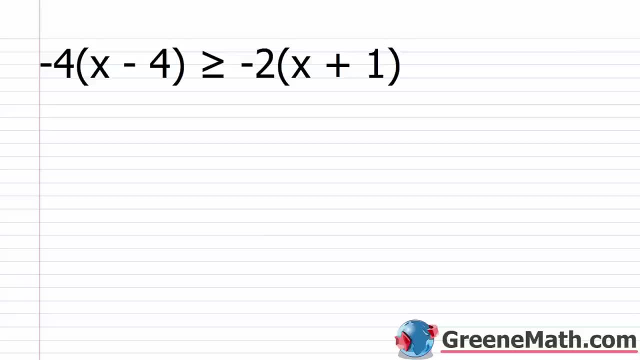 So we're just going to kind of jump in here. We already know the basics and so anything else that we're going to learn we're going to learn along the way. 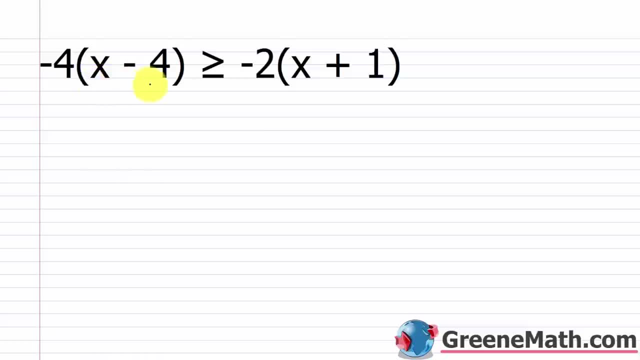 So when I look at this I have negative 4 times the quantity x minus 4 is greater than or equal to negative 2 times the quantity x plus 1. 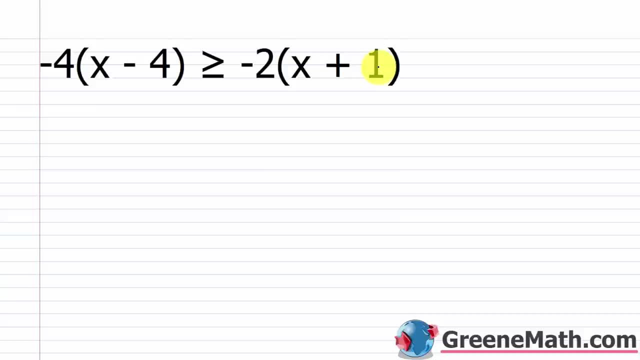 The same way I would do an equation, I'm going to simplify each side completely. So I'm going to use my distributive property on the left. Negative 4 times x is negative 4x. Then I have negative 4 times negative 4 that's plus 16. And this is greater than or equal to we have negative 2 times x that's negative 2x. 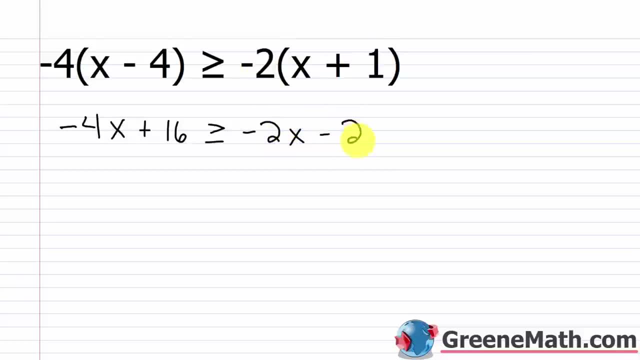 And then negative 2 times 1 that's minus 2. Now just like with an equation I want all my variable terms on one side of the inequality. And all my numbers on the other. So I can use my addition property of inequality to accomplish this. I can add 2x to both sides of the inequality. This will cancel. 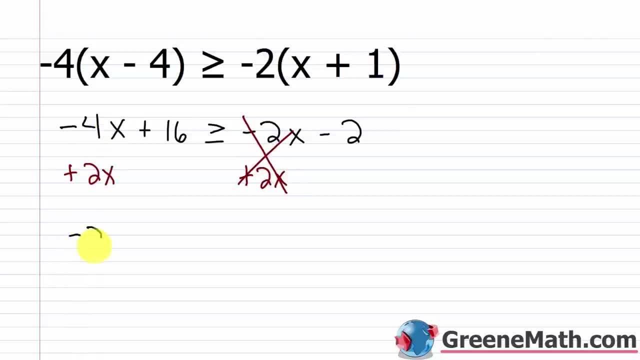 And let's see what we have. We have negative 4x plus 2x that's negative 2x. So then plus 16 is greater than or equal to negative 2. So now I just want to subtract 16 away from both sides of the inequality. So this can go away and my variable term is isolated. 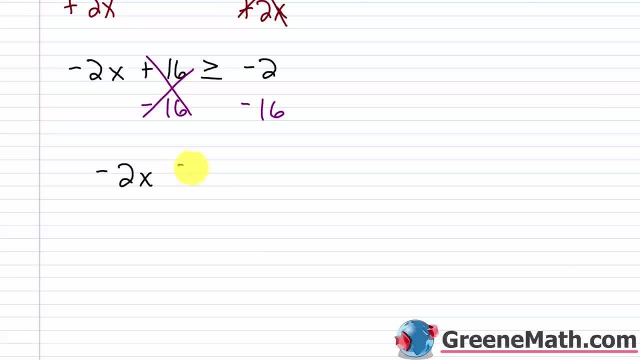 So now on the left I just have negative 2x. And then is greater than or equal to on the right 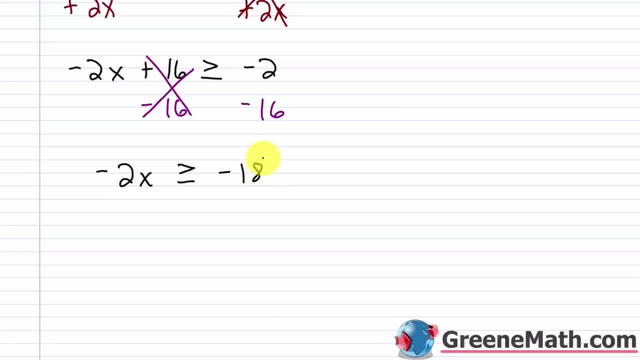 negative 2 minus 16 is negative 18. And I have one final step. I just want to isolate my variable x. 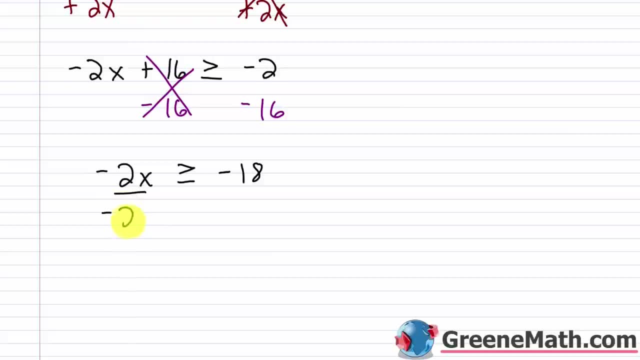 And so I'm going to divide both sides of the inequality by negative 2. 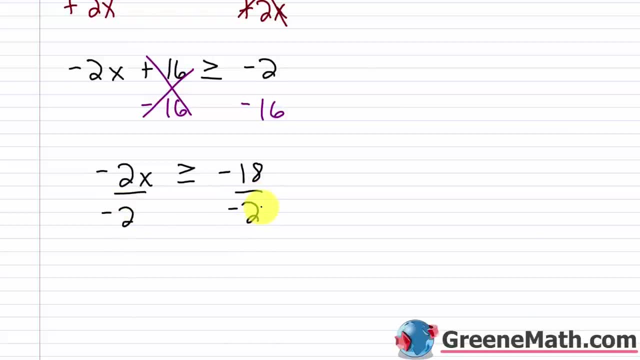 But remember we talked about this in the last lesson. 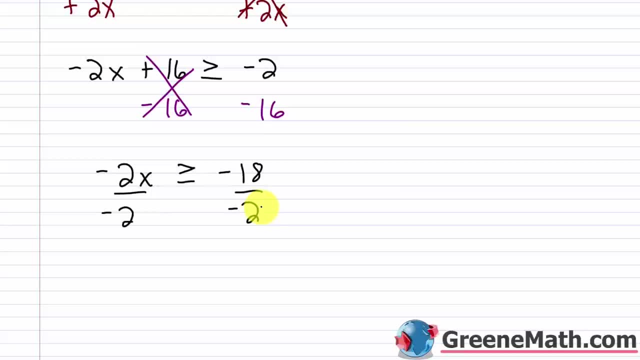 If you multiply or you divide by a negative you've got to flip the direction of the inequality. 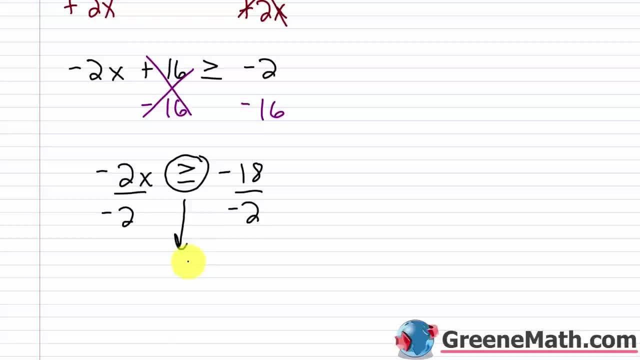 So right now this is a greater than or equal to we're going to make it a less than or equal to. 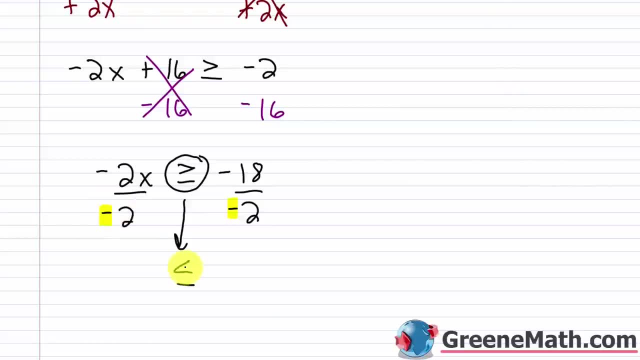 Again because we divided by a negative. Alright so once we've flipped it we don't have to do anything else. 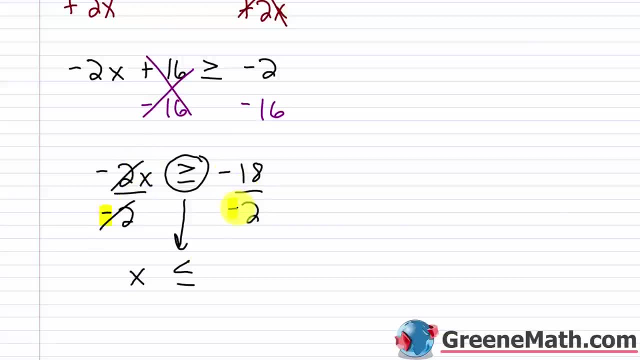 This cancels with this and we just have x. And on the right negative 18 divided by negative 2 is not. 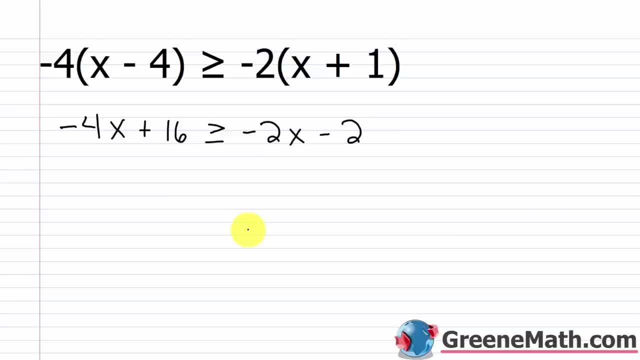 So I can use my addition property of inequality to accomplish this. I can add 2x to both sides of the inequality. This will cancel And let's see what we have. We have negative 4x plus 2x. That's negative 2x. 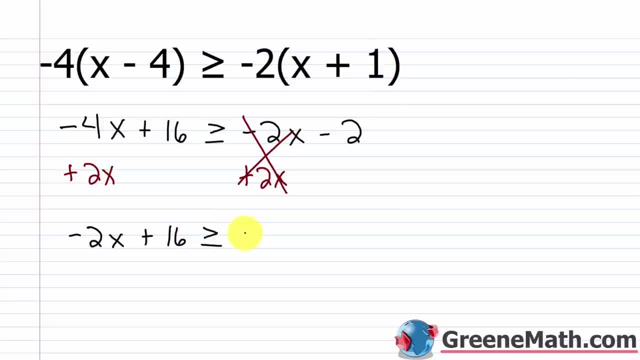 So then plus 16. Is greater than or equal to negative 2.. So now I just want to subtract 16 away from both sides of the inequality, So this can go away and my variable term is isolated. All right, So now, on the left, I just have negative 2x. 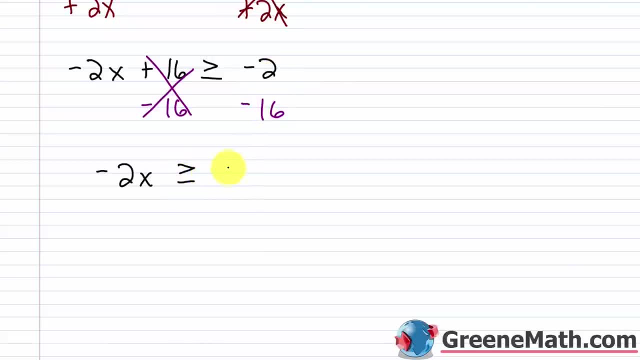 And then is greater than or equal to, On the right, negative 2 minus 16 is negative 18.. And I have one final step: I just want to isolate my variable x, And so I'm going to divide both sides of the inequality by negative 2.. 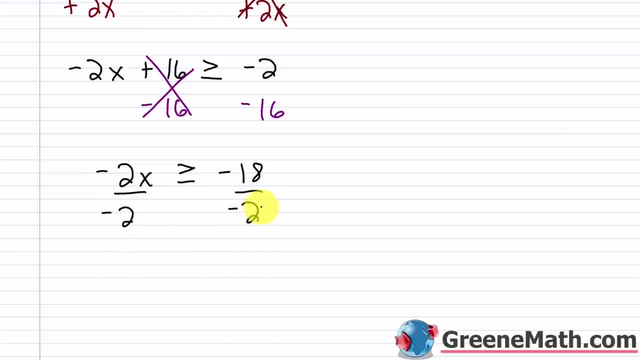 But remember- we talked about this In the last lesson- if you multiply or you divide by a negative, you've got to flip the direction of the inequality. So right now, this is a greater than or equal to. We're going to make it a less than or equal to. 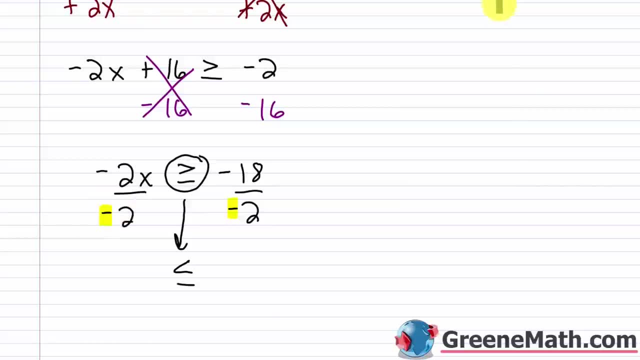 Again because we divided by a negative. All right, So once we flipped it, we don't have to do anything else. This cancels with this and we just have x. And on the right, negative 18 divided by negative 2 is not. 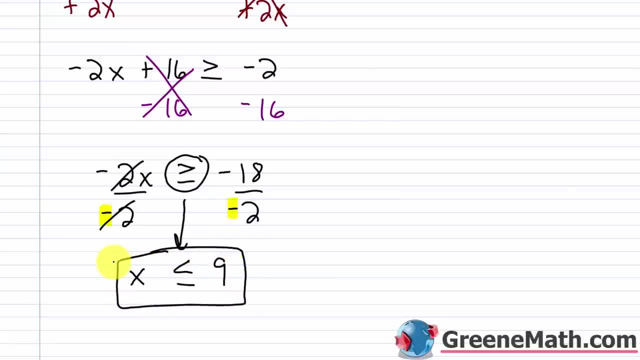 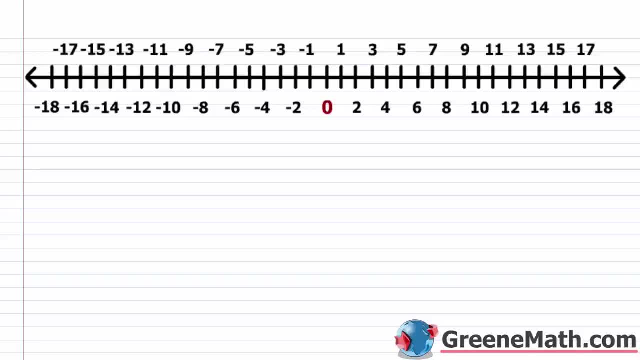 So our solution here is: x is less than or equal to 9.. Now, one thing we want to do when we're working with inequalities: we want to write our solution in what's known as interval notation. So we spent a lot of time on that in the last lesson. 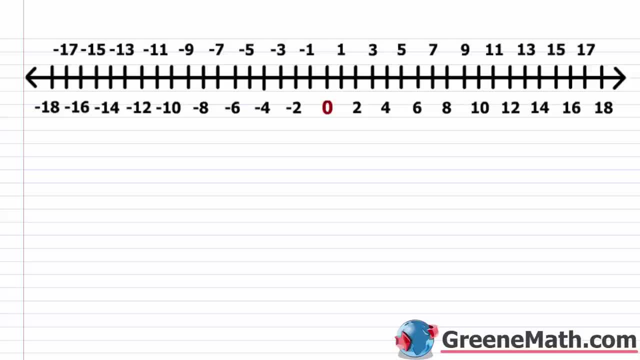 And so if you haven't covered that yet, I want you to go back to the last lesson and learn how to do that. So if we have, x is less than or equal to 9 in interval notation, remember it's less than or equal to 9.. 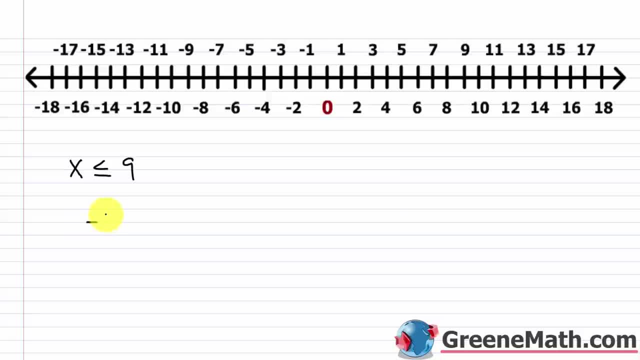 So the smallest value, there won't be one right, Because x could be 9.. So we're going to use negative infinity in that position. So we're going to use negative infinity in that position. And remember when we use positive infinity or negative infinity. So our solution here is x is less than 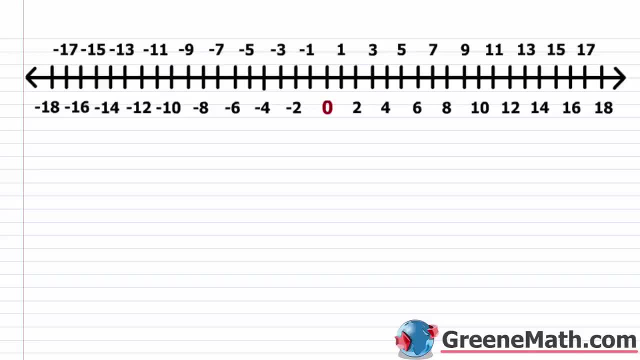 Now one thing we want to do when we're working with inequalities. We want to write our solution in what's known as interval notation. 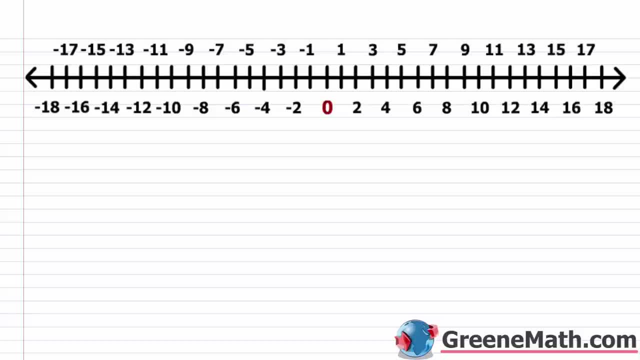 So we spent a lot of time on that in the last lesson. And so if you haven't covered that yet I want you to go back to the last lesson and learn how to do that. 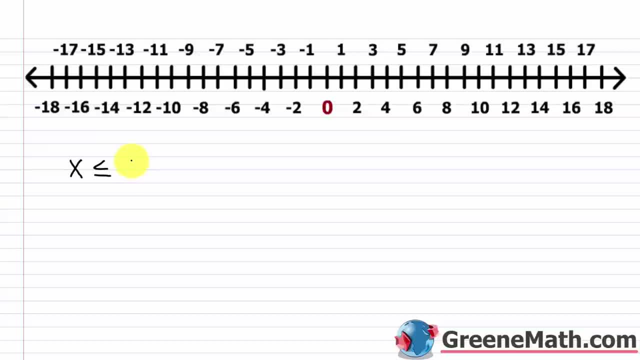 So if we have x is less than or equal to 9 in interval notation remember it's less than or equal to 9. So the smallest value 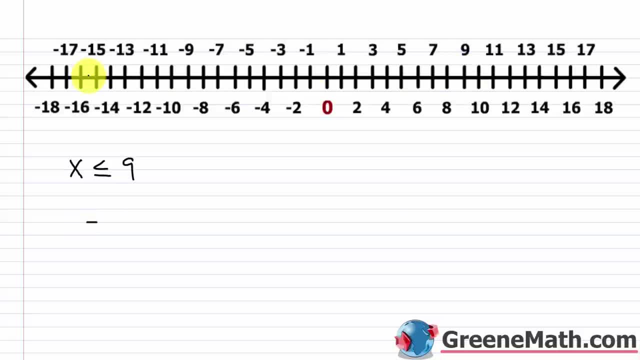 there won't be one. Because x could be 9 or anything less than that. So we're going to use negative infinity in that position. 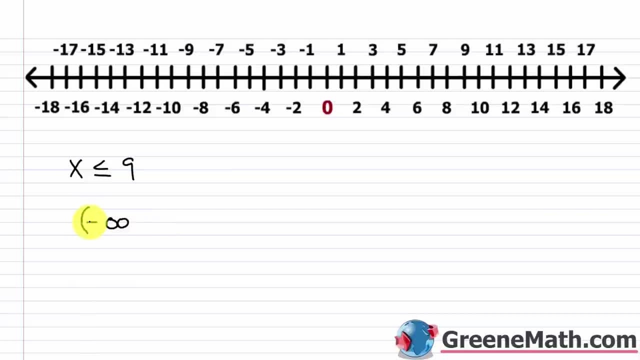 And remember when we use positive infinity or negative infinity we always put a parenthesis next to that. 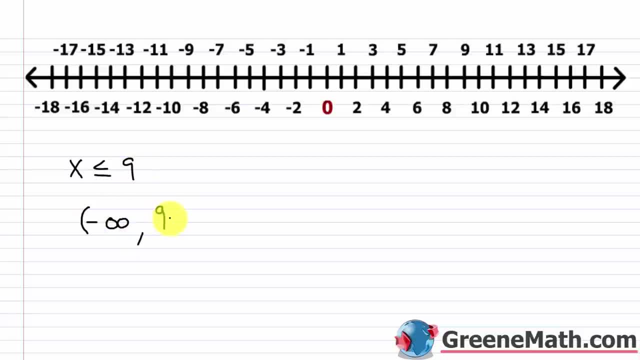 And then for the largest value we're going to use 9. 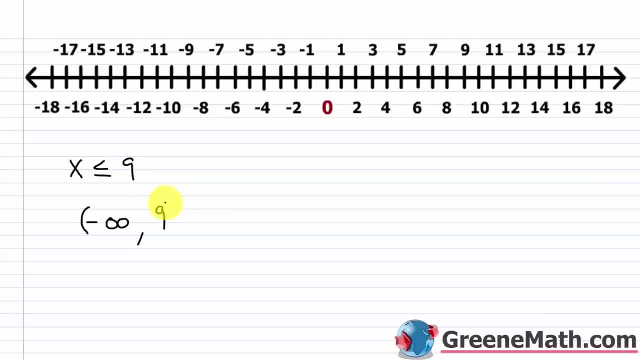 Now 9 is included in our solution and when something is included we're going to use a bracket not a parenthesis. 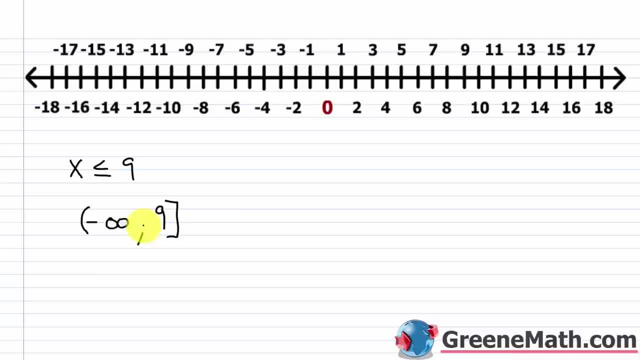 So we have our solution in interval notation 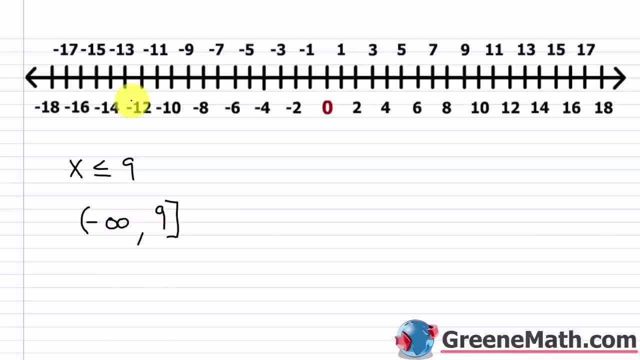 and then we just want to go ahead and graph it. 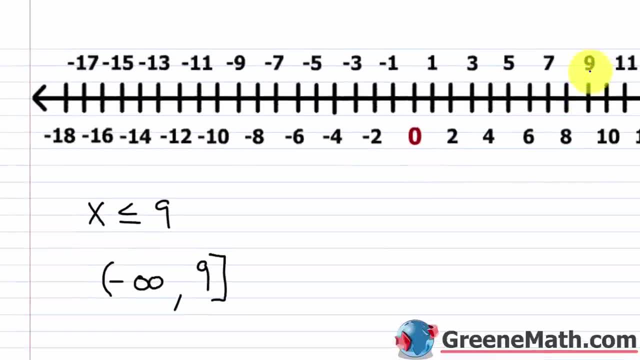 So we're going to locate 9 on our number line and 9 is right here. 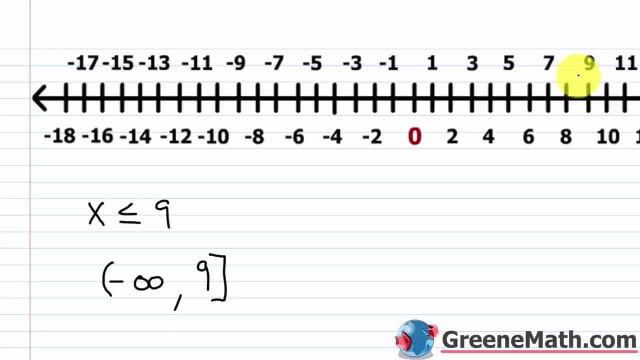 And I want to put a bracket at 9 that's facing to the left. It's always going to be facing in the direction of the solution. 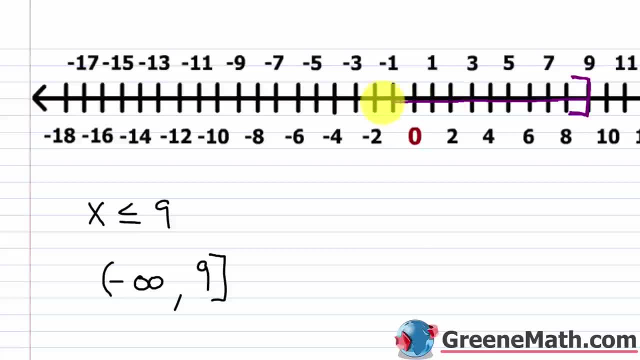 So the bracket goes there. And then I'm just going to shade everything to the left. Everything to the left. Shade all of that. Including the arrow. 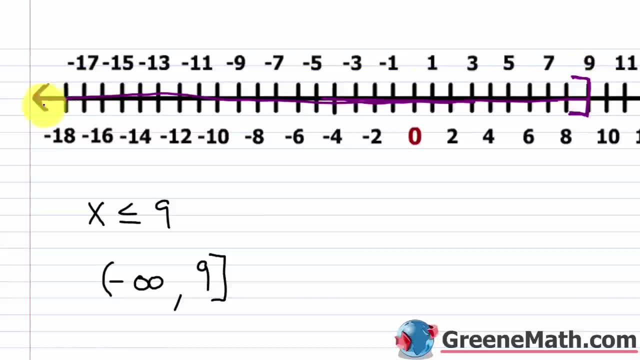 So x could be 9. That's why the bracket's there. Or anything to the left of 9 on the number line. 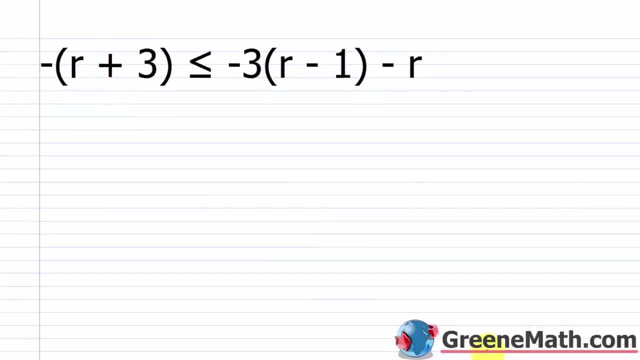 Alright, let's take a look at another one. We have the opposite of the quantity r plus 3. And this is less than or equal to negative 3 times the quantity r minus 1 and then minus r. 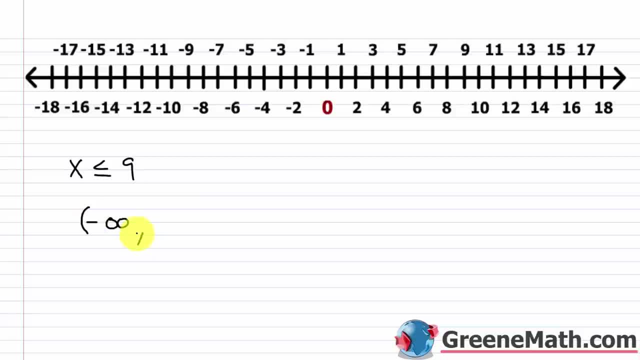 we always put a parenthesis next to that, And then, for the largest value, we're going to use 9.. Now, 9 is included in our solution, And when something's included, we're going to use a bracket, not a parenthesis. 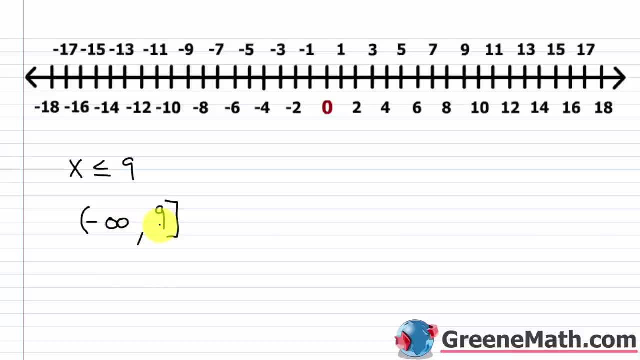 So we have our solution in interval notation And then we just want to go ahead and graph it. So we're going to look at the first one and then we're going to look at the second one. So we're going to look at the first one and then we're going to look at the second one. 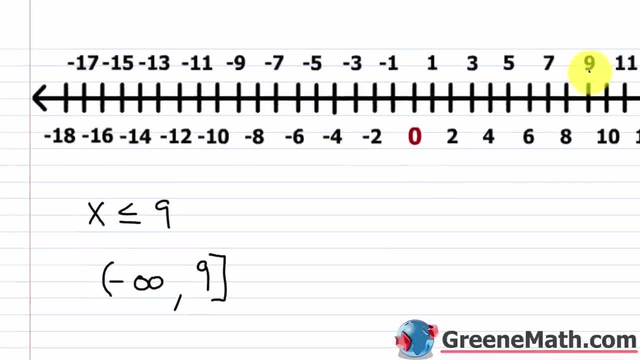 So we're going to locate 9 on our number line And 9 is right here And I want to put a bracket at 9. that's facing to the left. It's always going to be facing in the direction of the solution. 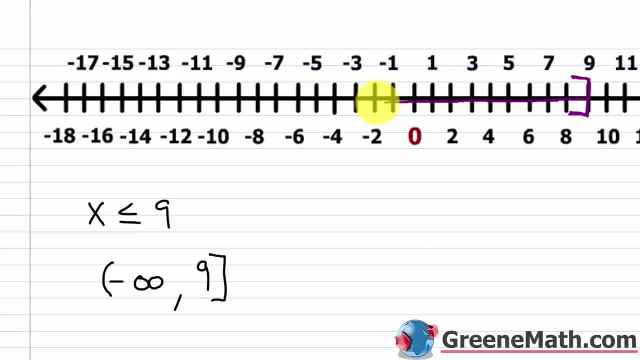 So the bracket goes there And then I'm just going to shade everything to the left, Everything to the left. Shade all of that including the arrow. So x could be 9.. That's why the bracket's there, Or anything to the left of 9 on the number line. 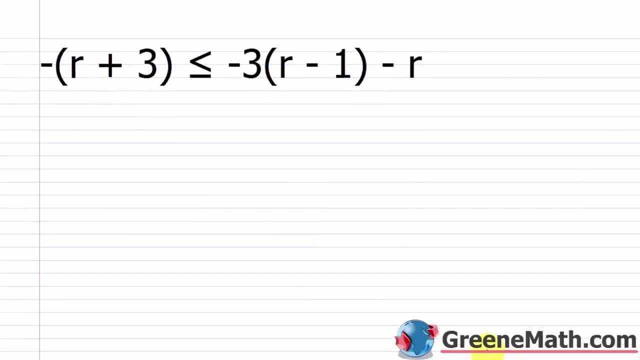 All right, let's take a look at another one. We have the opposite of the quantity r plus 3.. And this is less than or equal to negative 3 times the quantity r minus 1, and then minus r. So I'm going to use my distributive property here. 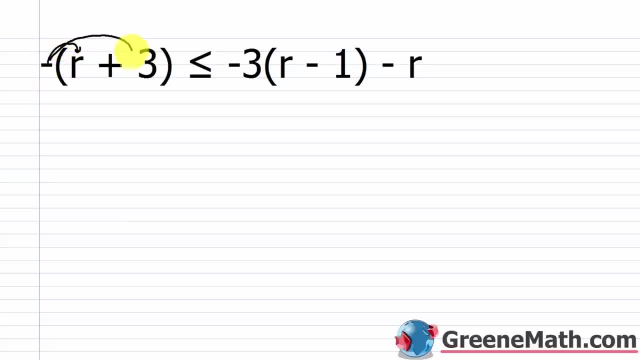 I'm going to distribute this negative to each term And remember you could put that as plus negative 1.. And think about that as okay. I'm multiplying negative 1 times r, That's negative r, And then negative 1 times 3.. 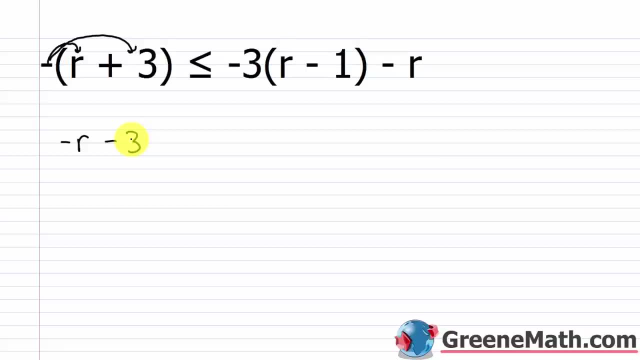 That's minus 3.. You can also just change the sign of each term inside the parentheses. That will allow you to remove the parentheses. Remember, if I see just a negative out in front of parentheses, in order to remove the parentheses, I change the sign of each term inside. 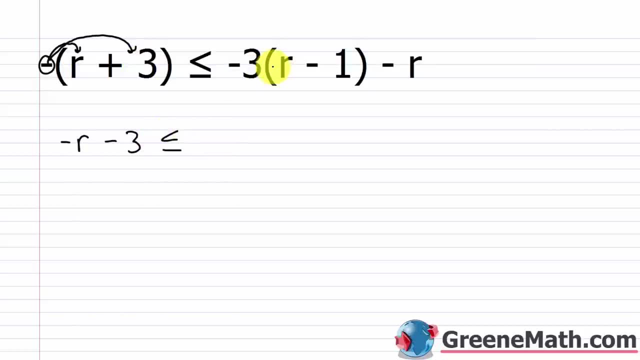 So negative r minus 3 is less than or equal to negative 3 times r, is negative 3r. And then negative 3 times negative 1 is plus 3.. And then minus r. All right, so let's continue simplifying. 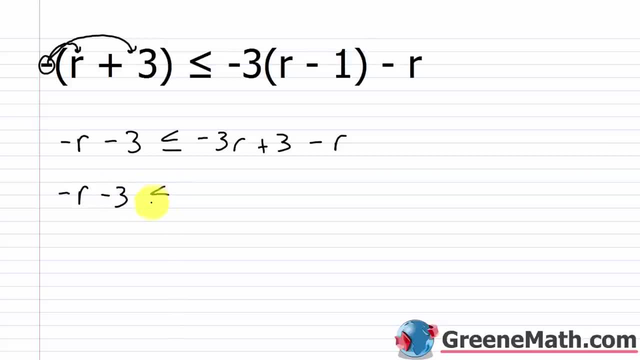 On the left, I have negative r minus 3.. This is less than or equal to. On the right, I have negative 3r minus r. I can combine those like terms That'll give me negative 4r and then plus 3.. 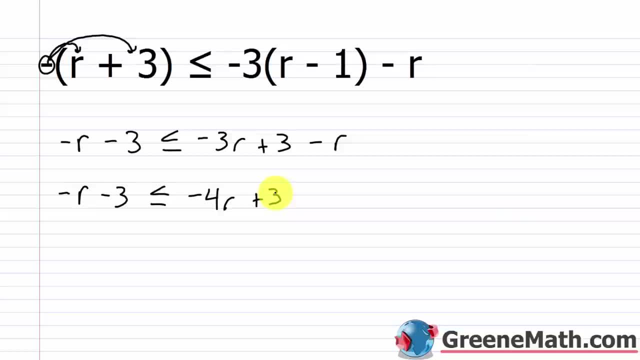 And now I want to move all the variable terms to one side and have the numbers on the other. So what I'm going to do is I'm going to add 4r to both sides of the inequality. So this is going to go away. 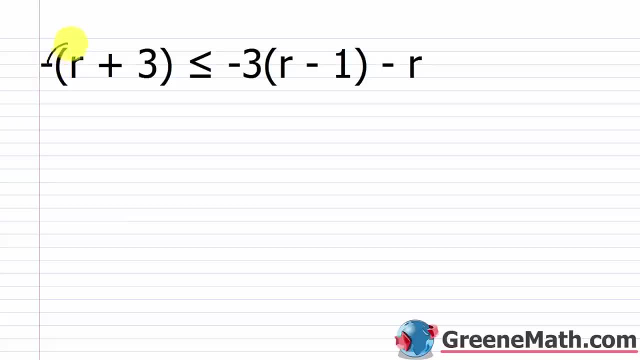 So I'm going to use my distributive property here. I'm going to distribute this negative to each term. And remember, you could put that as plus negative 1 and think about that as multiplying negative 1 times r. That's negative r. And then negative 1 times 3. That's minus 3. You can also just change the sign of each term inside the parentheses. 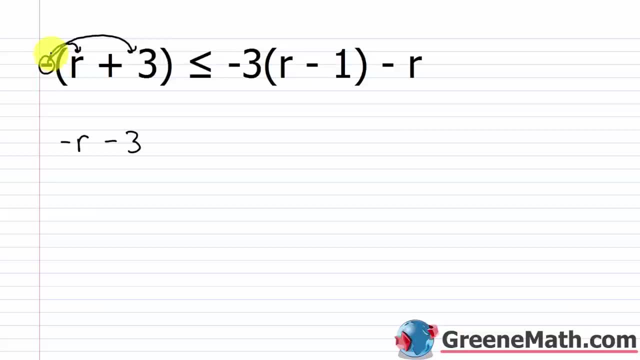 That will allow you to remove the parentheses. Remember, if I see just a negative out in front of parentheses in order to remove the parentheses I change the sign of each term inside. So negative r minus 3 is less than or equal to negative 3 times r is negative 3r and then negative 3 times negative 1 is plus 3 and then minus r. 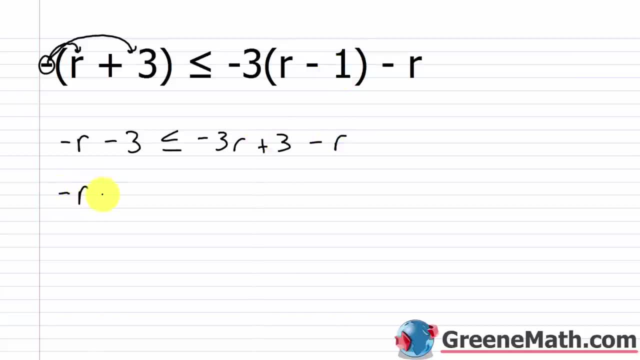 Alright, so let's continue simplifying. On the left I have negative r minus 3 and this is less than or equal to on the right I have negative 3r minus r I can combine those like terms that will give me negative 4r and then plus 3. And now I want to move all the variable terms to one side and have the numbers on the other. 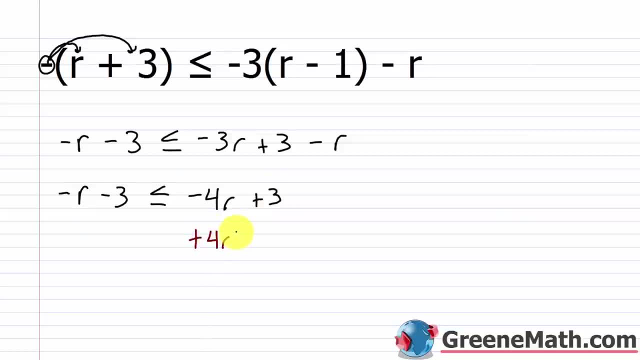 So what I'm going to do is I'm going to add 4r to both sides of the inequality. So this is going to go away. 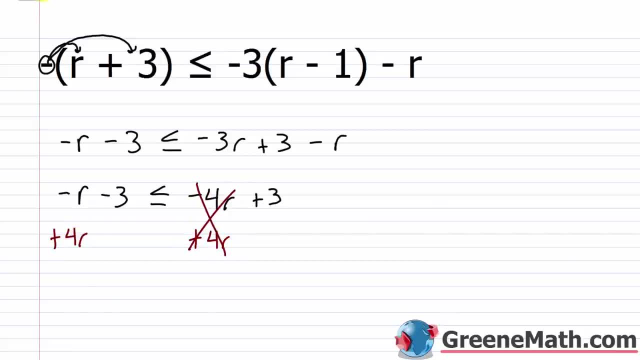 And negative r plus 4r would be 3r. 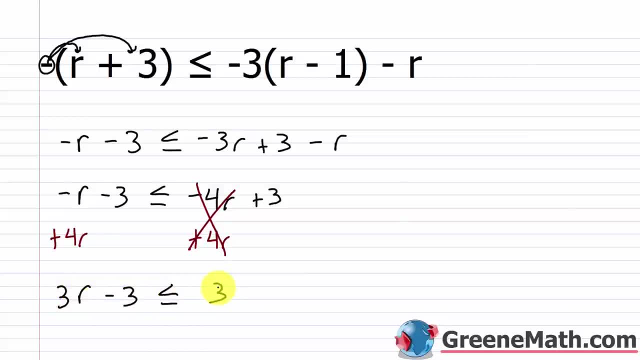 So then minus 3 is less than or equal to 3. 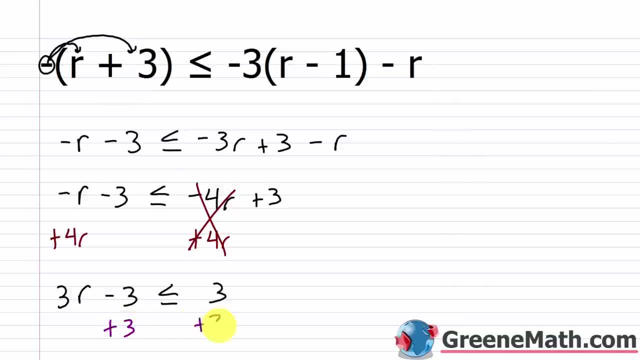 And now I'm simply going to add 3 to both sides of the inequality. So that I can isolate this 3r. 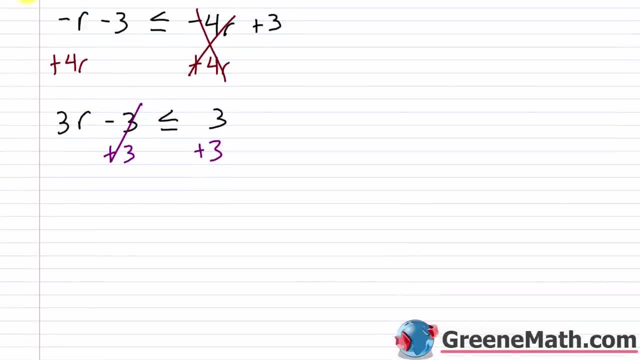 So this will go away. And on the left I'll just simply have 3r now. 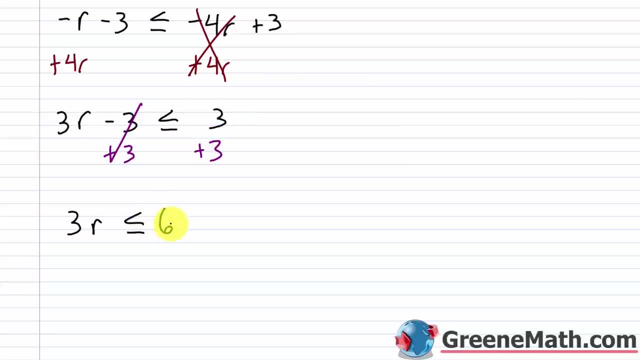 This is less than or equal to 3 plus 3 is 6. 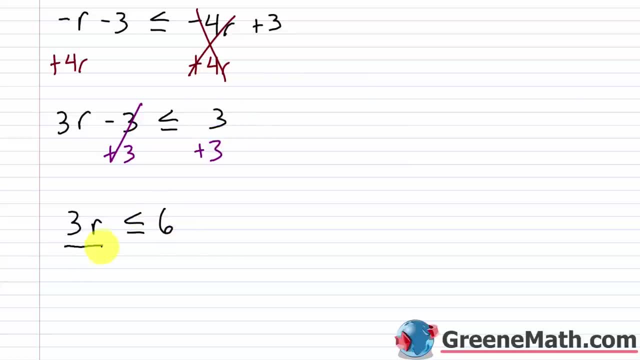 Now as a final step I'm going to divide both sides of the inequality by 3. Which is the coefficient of r. 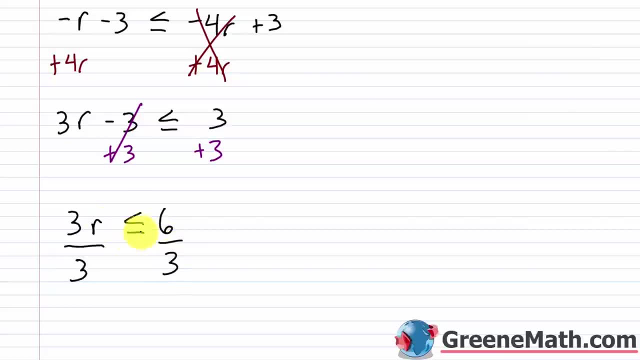 Now again because I'm dividing by a positive number I don't need to do anything with the sign. 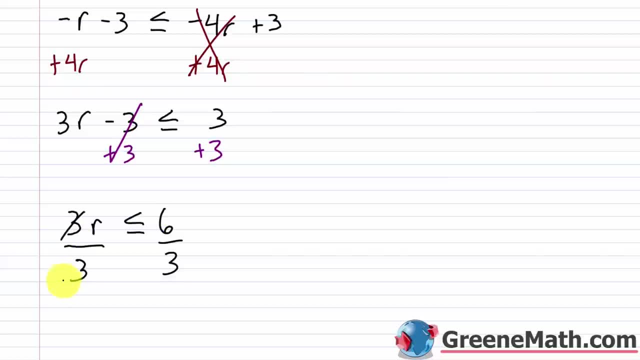 It's only if I'm doing it with a negative number. So this will cancel with this. 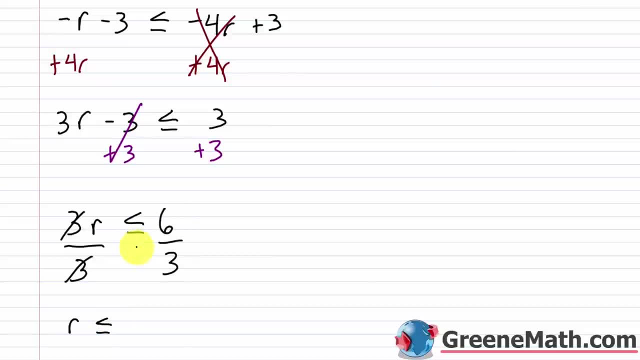 I'll have r and then is less than or equal to 6 divided by 3 is 2. So r is less than or equal to 2. Alright so in interval notation again we have r is less than or equal to 2. 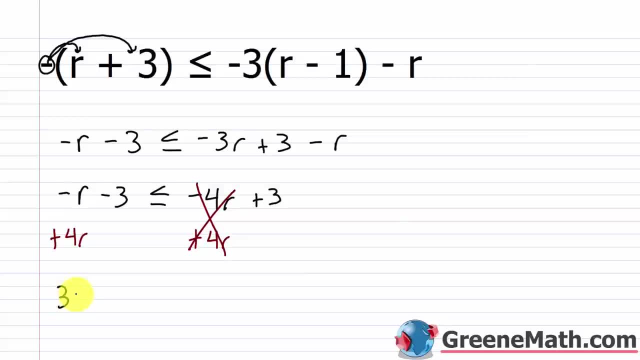 And negative r plus 4r would be 3r. So then minus 3 is less than or equal to 3.. And now I'm simply going to add 3 to both sides of the inequality So that I can isolate this 3r. 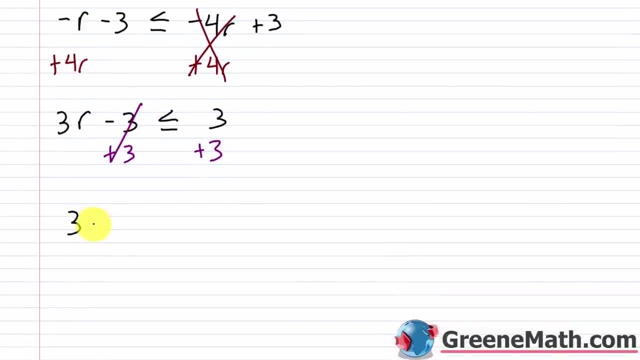 So this will go away, And on the left, I'll just simply have 3r. now. This is less than or equal to, 3 plus 3 is 6.. Now, as a final step, I'm going to divide both sides of the inequality by 3,. 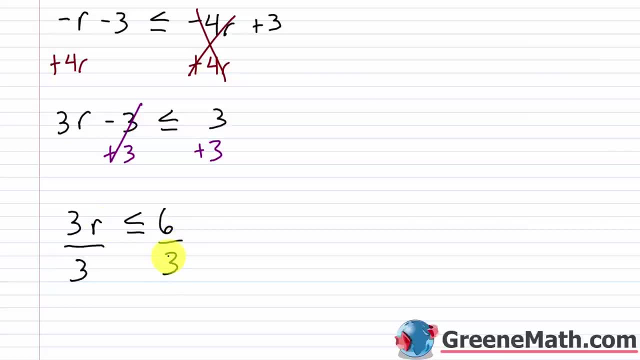 which is the coefficient of r. Now again, because I'm dividing by a positive number, I don't need to do anything with the sign. It's only if I'm doing it with a negative number. So this will cancel. with this I'll have r, and then is less than or equal to. 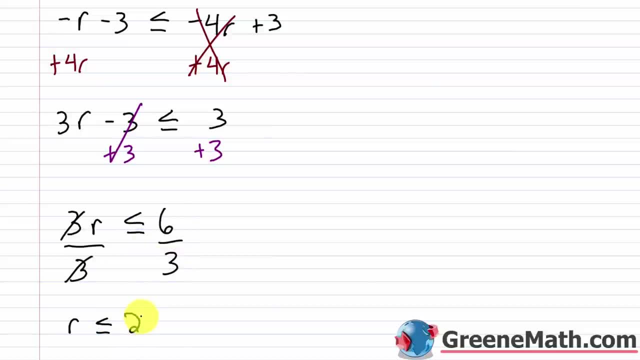 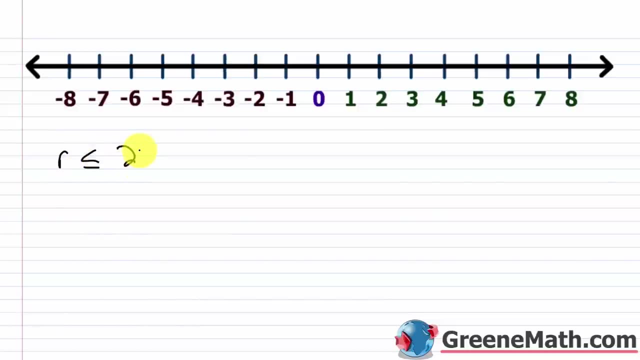 6 divided by 3 is 2.. So r is less than or equal to 2.. All right, So an interval notation. Again we have: r is less than or equal to 2.. So that's going to look like this: 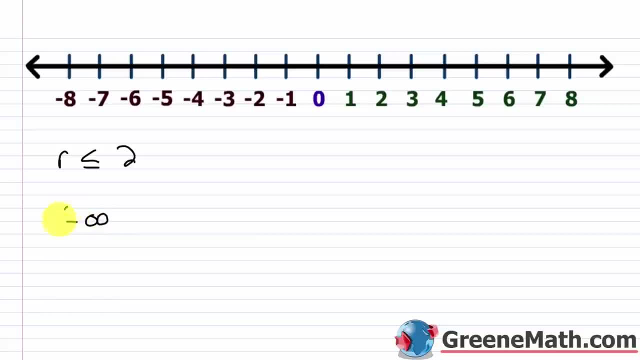 We'd have negative infinity right here. We put a parenthesis there to say that negative infinity is not included, And then this is up to and including 2, right, So we're going to use a bracket at 2.. Because r can be anything kind of starting out at 2,. 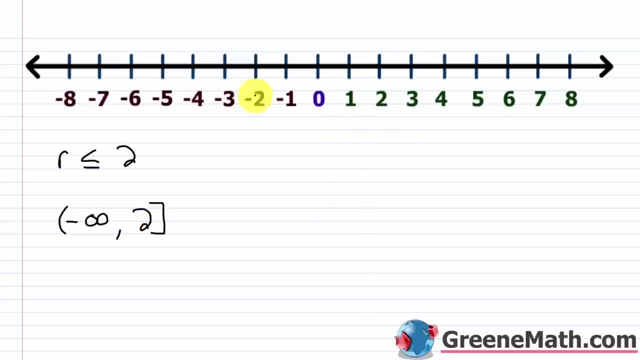 including 2, anything moving to the left. So the smallest possible value? there's not one. That's why we put negative infinity here. The largest possible value is 2. And 2 is included. So we put our bracket. Now again, when we graph this, we put a bracket at 2, facing to the left. 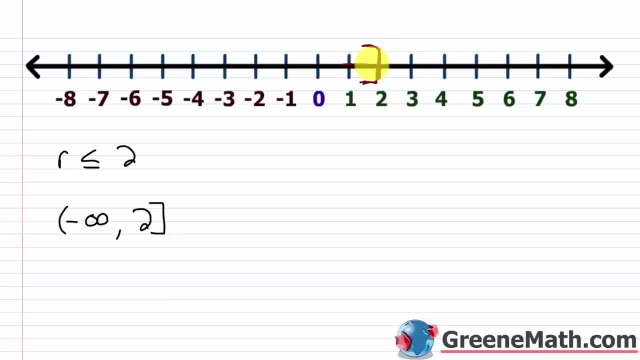 It's facing towards the solution, And then we're going to highlight or we're going to shade everything to the left, including this arrow, to say, hey, 2 is included, And everything to the left of 2 is included as a solution as well. 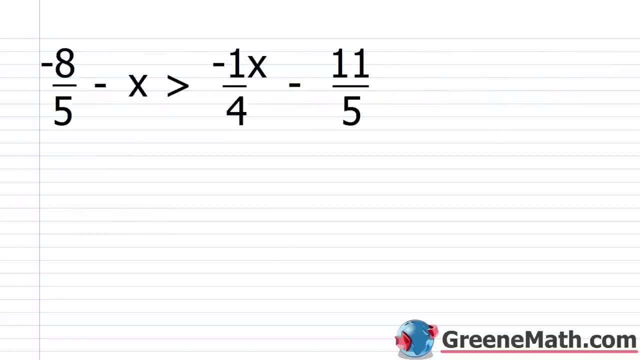 All right, let's take a look at another one. We have negative: 8 fifths minus x is greater than negative 1 fourth x minus 11 fifths. So, just like if we had an equation with fractions, if we have an inequality with fractions. 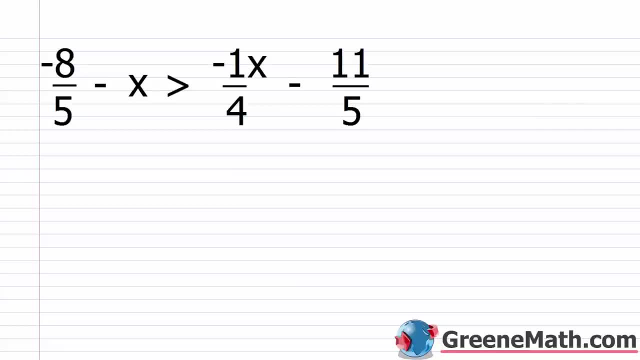 we can go ahead and multiply both sides of the inequality by the LCD. So the LCD here would be 20, right 5 times 4.. I can multiply 20 times the left side, which is negative 8 fifths minus x. 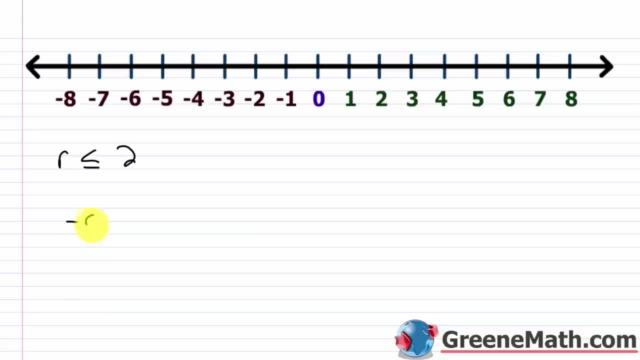 So that's going to look like this. We'd have negative infinity right here. We'll put a parenthesis there to say that negative infinity is not included. And then this is up to and including 2. Alright so we're going to use a bracket at 2. Because r can be anything kind of starting out at 2 including 2 anything moving to the left. 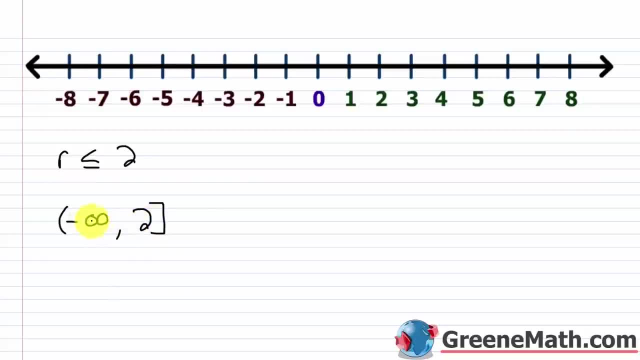 So the smallest possible value there's not one. That's why we put negative infinity here. 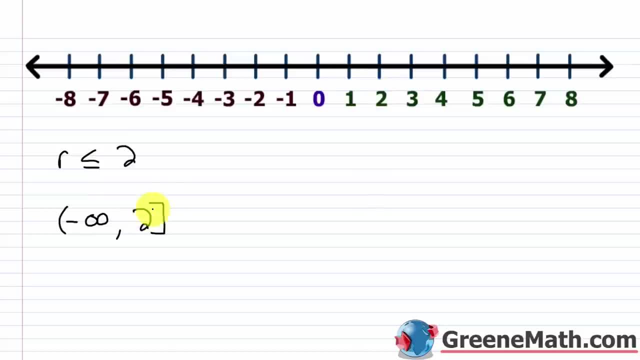 The largest possible value is 2. And 2 is included. So we put our bracket. 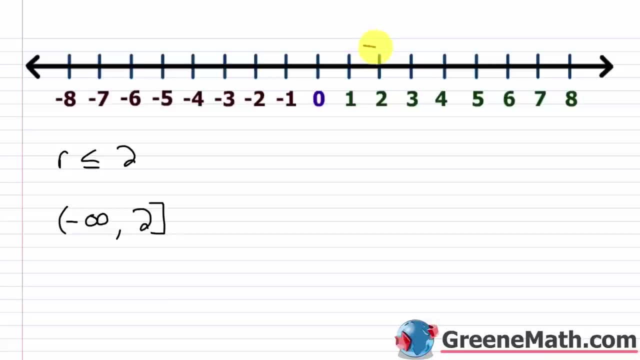 Now again when we graph this we put a bracket at 2 facing to the left. It's facing towards the solution. 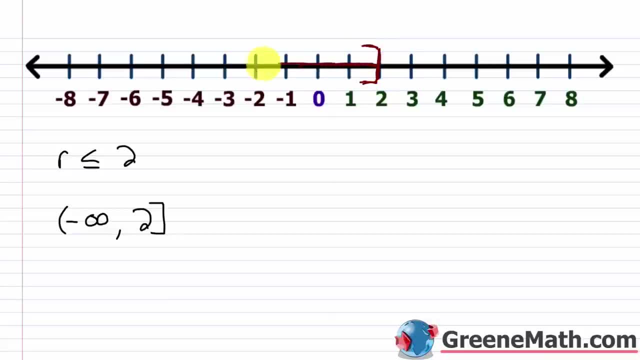 And then we're going to highlight or we're going to shade everything to the left including this arrow to say hey 2 is included and everything to the left of 2 is included as a solution as well. 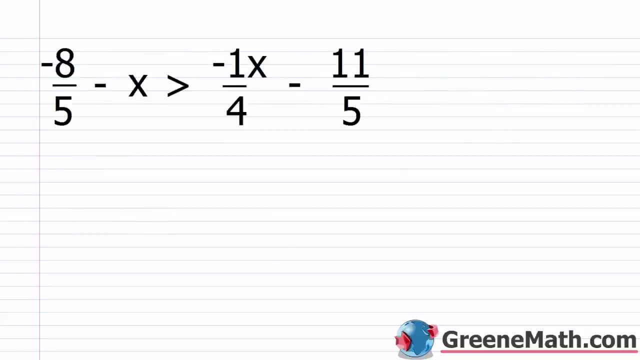 Alright let's take a look at another one. We have negative 8 fifths minus x is greater than negative 1 fourth x minus 11 fifths. So just like if we had an equation with fractions if we have an inequality with fractions we can go ahead and multiply both sides of the inequality by the LCD. 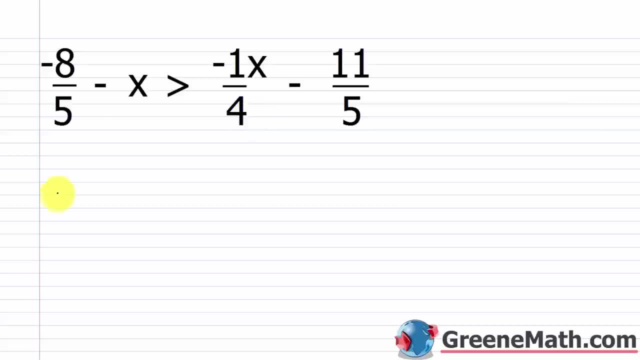 So the LCD here would be 20. 5 times 4. So I can multiply 20 times the left side which is negative 8 fifths minus x. Remember to use brackets or parentheses. You've got to multiply 20 by both. This is greater than negative 1 fourth times x minus 11 fifths. We're multiplying everything over here by 20 as well. 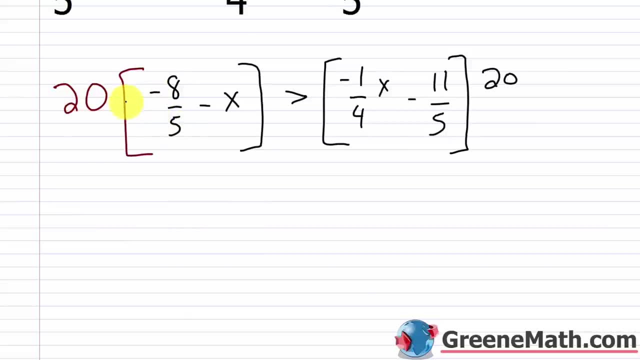 So 20 times negative 8 fifths 20 we cancel with 5 and give me 4. 4 times negative 8 is negative 32. 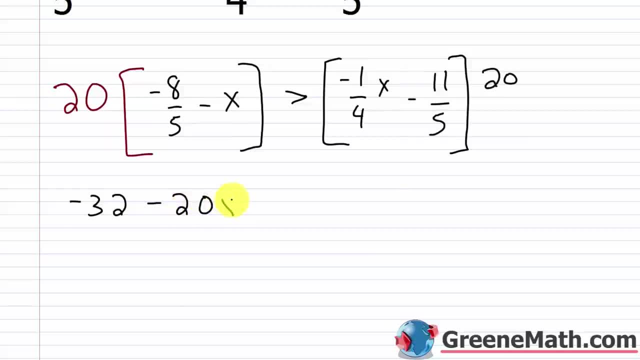 So then minus 20 times x is 20x. And this is greater than over here 20 times negative 1 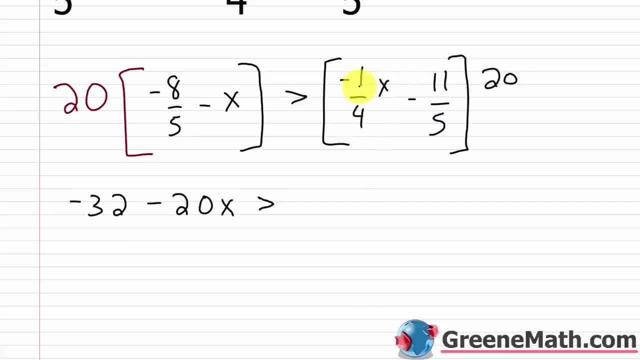 fourth x. So 20 divided by 4 is 5. 5 times negative 1 is negative 5. So this would be negative 5x. 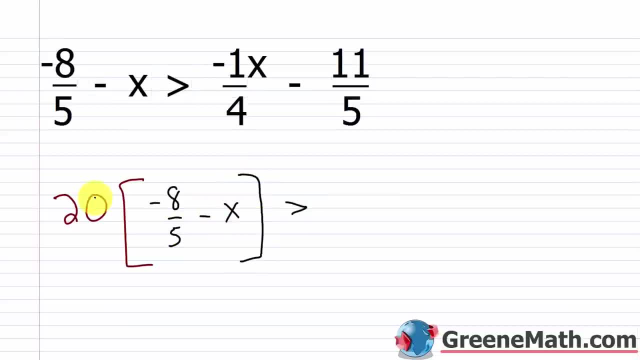 Remember to use brackets or parentheses. right, You've got to multiply 20 by both terms. This is greater than I'm going to use brackets over here. negative 1 fourth times x minus 11 fifths. We're multiplying everything over here by 20 as well. 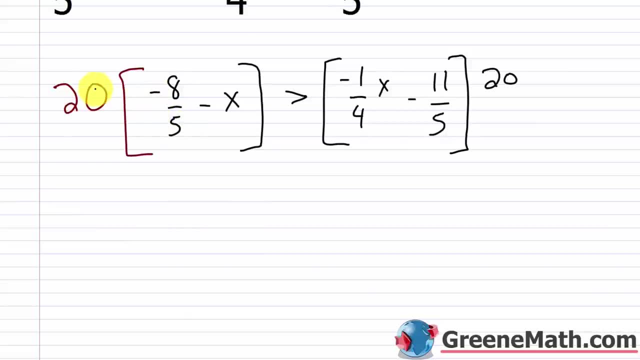 So 20 times negative 8, fifths 20, we cancel with 5 and give me 4.. 4 times negative 8 is negative 32.. So then, minus 20 times x is 20x, And this is greater than over here. 20 times negative 1. fourth x. 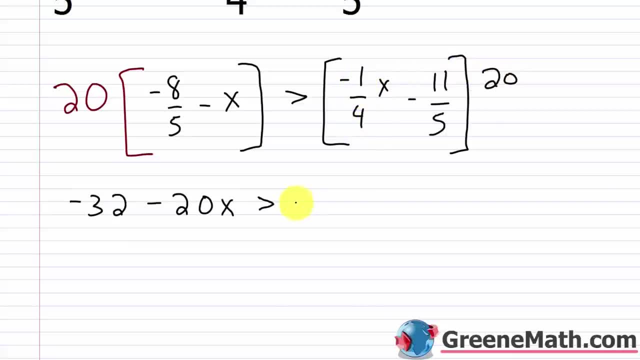 So 20 divided by 4 is 5.. 5 times negative 1 is negative 5.. So this would be negative 5x. And then minus 20 divided by 5 would be 4.. 4 times 11 is 44.. 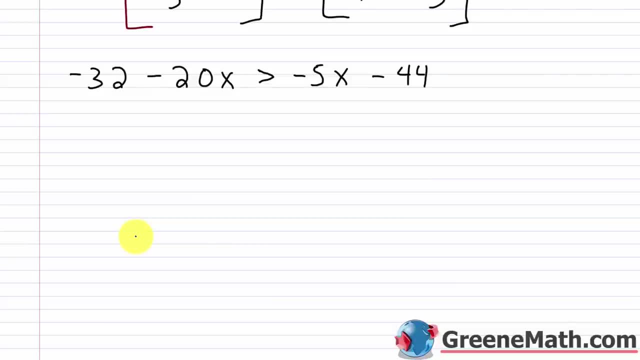 All right. so I want to get my variable term on one side of the inequality and a number on the other. So I'm going to add 5x to both sides of the inequality. That's going to go away, And on the left side I'm going to have negative 32.. 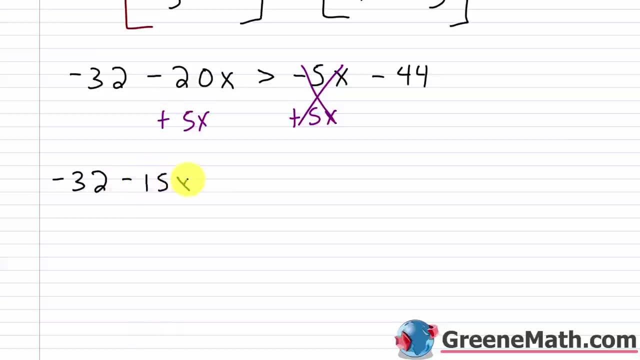 Negative 20x plus 5x is minus 15x. This is greater than negative 44. So then the next step is to add 32 to both sides of the inequality, So that'll cancel And I'll have negative 15x. 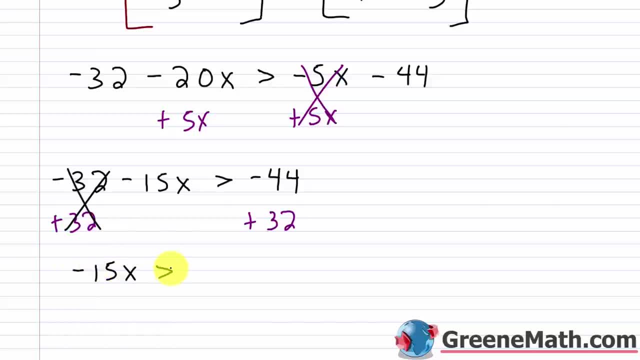 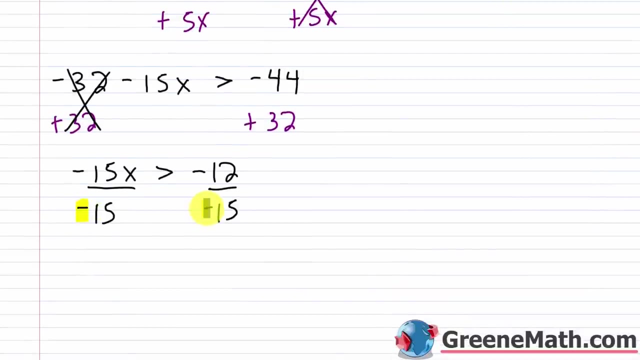 It's greater than negative. 44 plus 32 is negative 12.. And as a final step, I'm going to divide both sides of the inequality by negative 15, which is the coefficient of x. Again, again, again, When I divide by a negative and I'm working with inequalities. 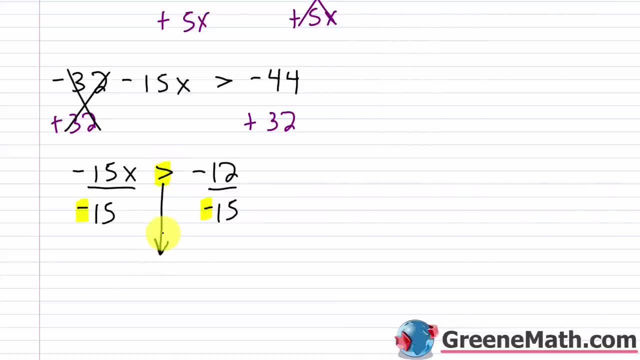 I've got to flip the direction of the inequality, So this is going to get flipped. Right now it's a greater than. We're going to make it a less than. So this would be that x right, because these are going to cancel. 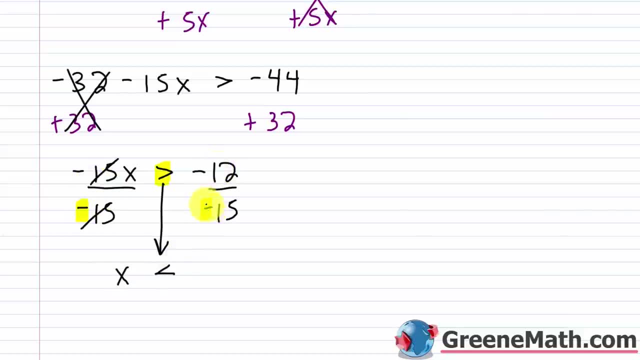 is less than negative. 12 over negative 15.. That's positive, Really. think about 12 as 4 times 3, and 15 is 5 times 3.. So the GCF would be 3.. Cancel that between numerator and denominator and you're going to get 4 fifths. 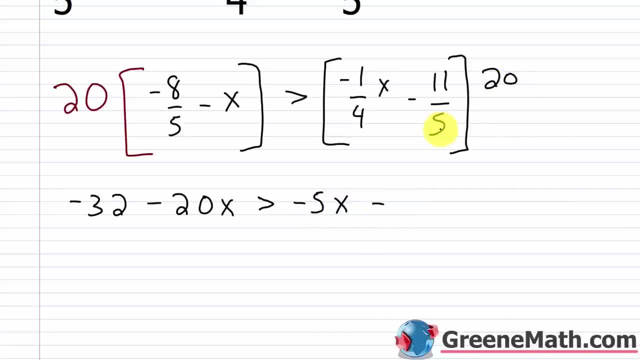 And then minus 20 divided by 5 would be 4. 4 times 11 is 44. 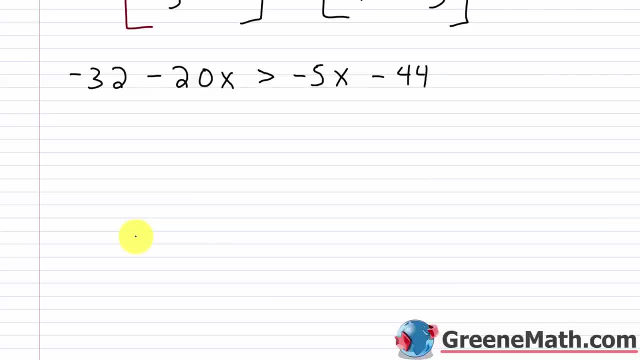 Alright, so I want to get my variable term on one side of the inequality and a number on the other. 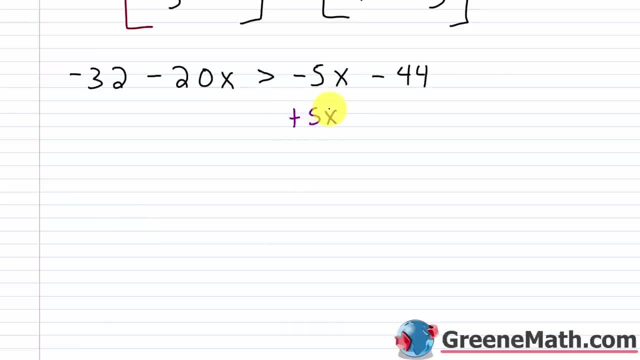 So I'm going to add 5x to both sides of the inequality. 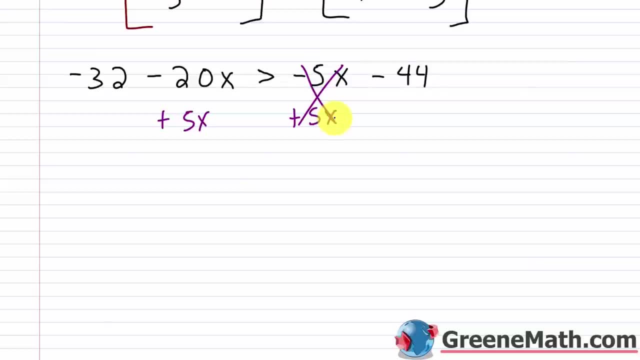 That's going to go away. 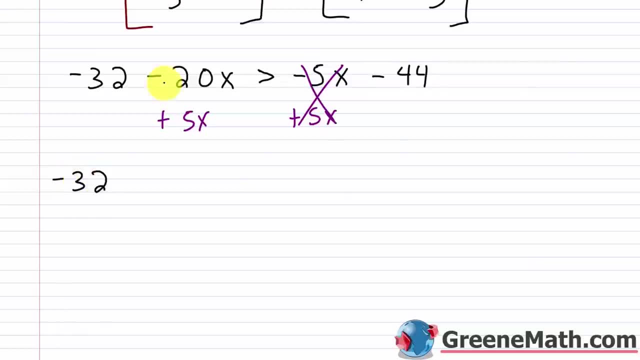 And on the left side I'm going to have negative 32. Negative 20x plus 5x is minus 15. This is greater than negative 44. So then the next step is to add 32 to both sides of the inequality. 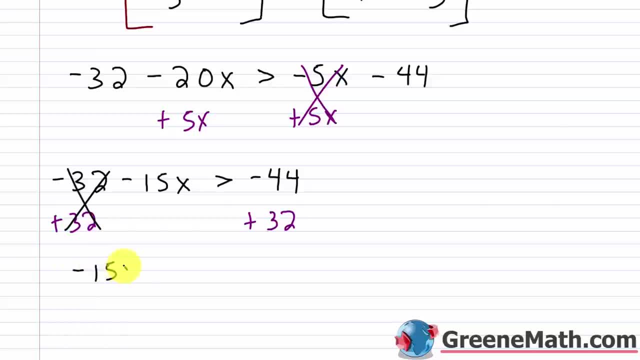 So that'll cancel. And I'll have negative 15x is greater than negative 44 plus 32 is negative 12. 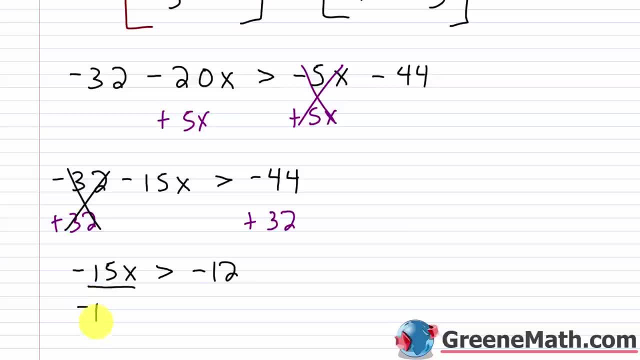 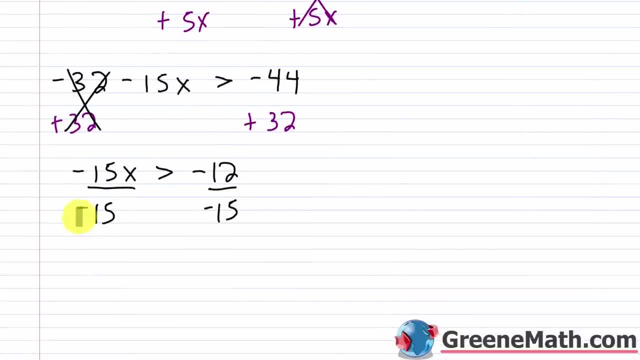 And as a final step I'm going to divide both sides of the inequality by negative 15, which is the coefficient of x. Again, I get it again. When I divide by a negative, and I'm working with inequalities, I've got to flip the direction of the inequality. So this is going to get flipped. Right now it's a greater than. We're going to make it a less than. 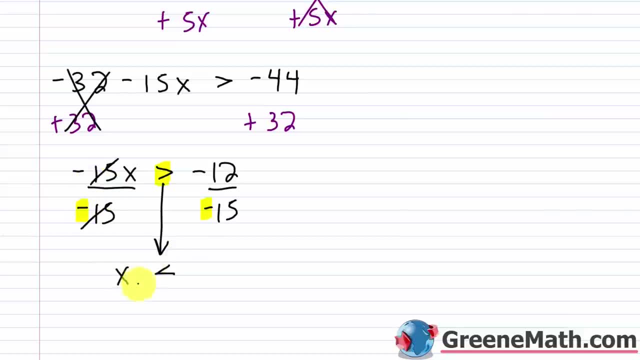 So this would be that x, because these are going to cancel, is less than negative 12 over negative 15. That's positive. Really think about 12 as 4 times 3. And 15 is 5 times 3. So the GCF would be 3. Cancel that between numerator and denominator. And you're going to get 4 fifths. 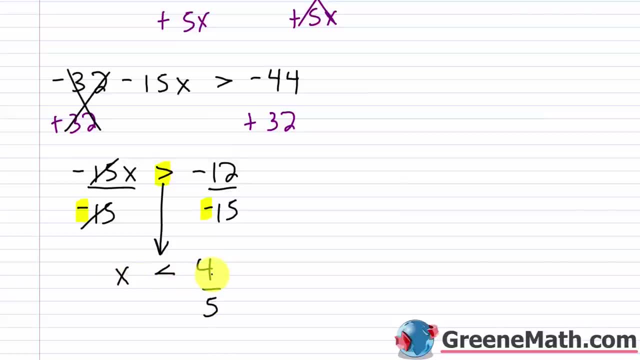 So we'd have x is less than 4 fifths. 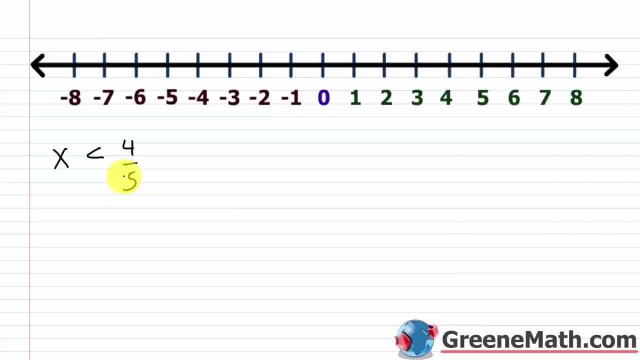 Alright, so let's write this in interval notation. So since x is less than 4 fifths, really for 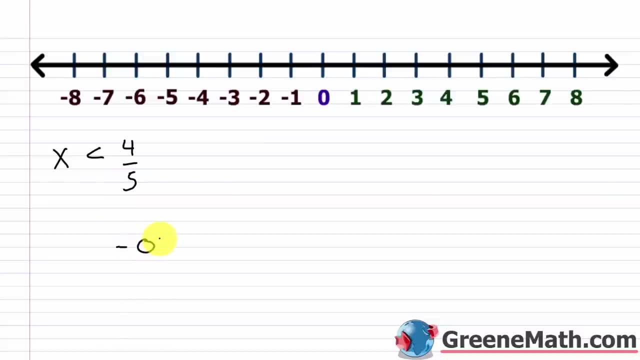 the smallest value we're going to put negative infinity. Because this is going to keep going forever and ever and ever in the left direction. So we'll put a parenthesis next to that. 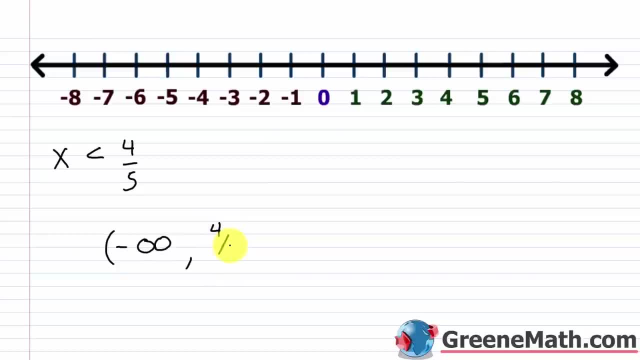 And then for the largest number we're going to put 4 fifths. And remember that's not included, because we have a strict inequality. So we're going to use a parenthesis there as well. 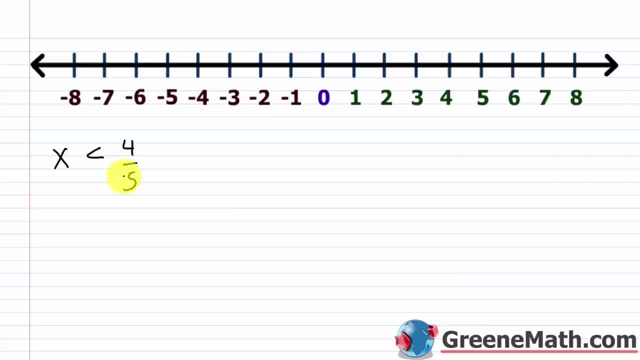 So we'd have: x is less than 4 fifths. All right, so let's write this in interval notation: So, since x is less than 4 fifths, really for the smallest value, we're going to put negative infinity Right, because this is going to keep going forever and ever and ever in the left direction. 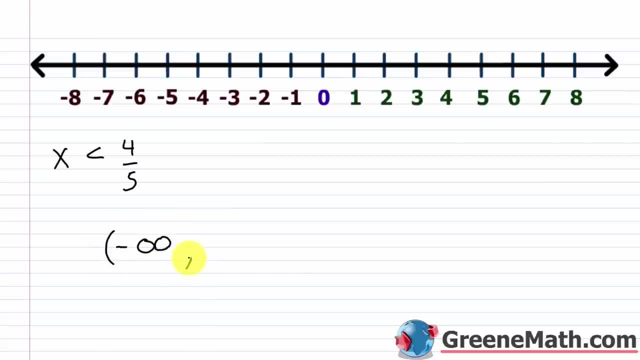 So we'll put a parenthesis next to that And then for the largest number we're going to put 4 fifths. And remember that's not included because we have a strict inequality, So we're going to use a parenthesis there as well. 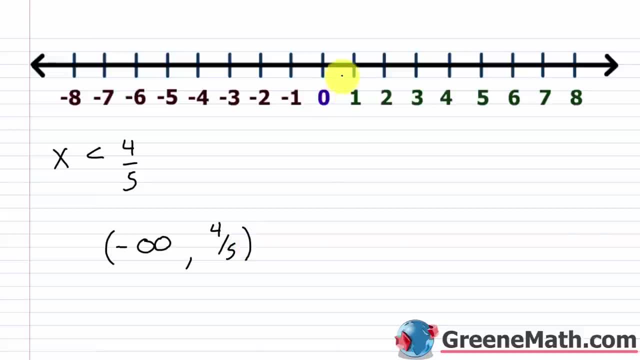 Now, graphically, we don't have a notch for 4 fifths, But let's say it's somewhere right there. Let's say this is 4 fifths. I'll put the notch there, And so I'm going to use a parenthesis at 4 fifths. 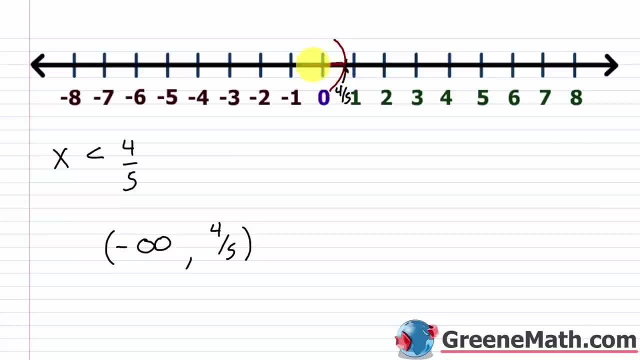 It's going to face to the left And I'm going to shade everything to the left, including this arrow right here. So that would be: x is less than 4 fifths. All right, let's take a look at another one with some fractions. 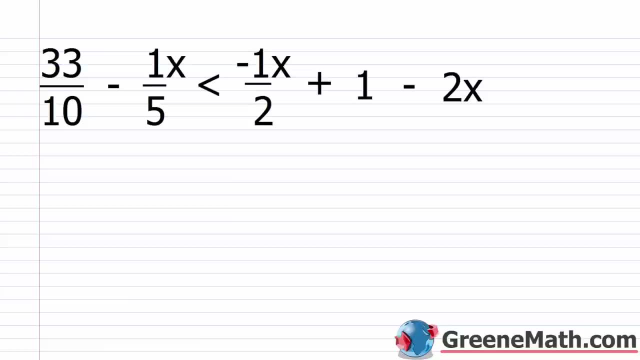 We have 33 tenths minus 1. fifth x is less than negative: 1 half x plus 1 minus 2 x. So the first thing I'm kind of looking at here is to clear the fractions. the LCD is 10.. All right, 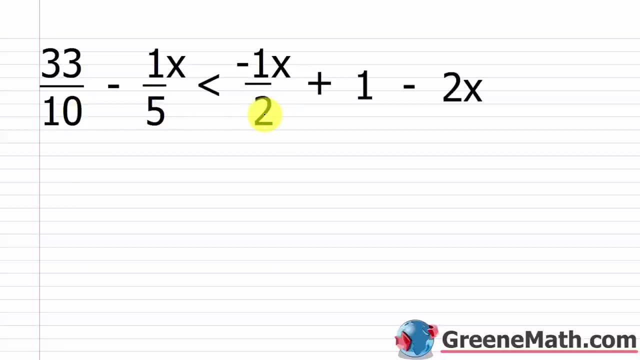 I have 5.. I have 2. And I have 10.. 5 times 2 is 10., So the LCD is 10.. So let's multiply both sides of the inequality by 10. So I'd have 10 times. 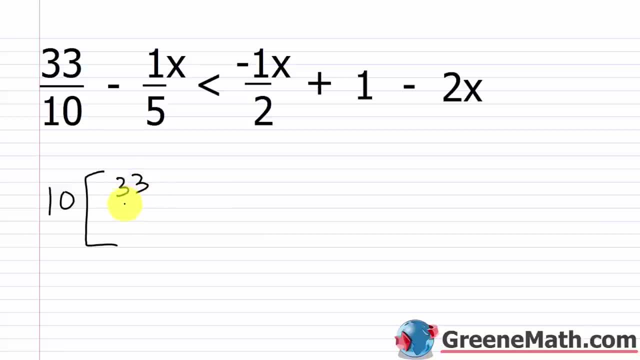 Remember to use brackets Or again, you could use parentheses if you want. So 33 over 10 minus 1 fifth times x. Close the brackets And then this is less than Open brackets. Negative: 1 half times x plus 1 minus 2 x. 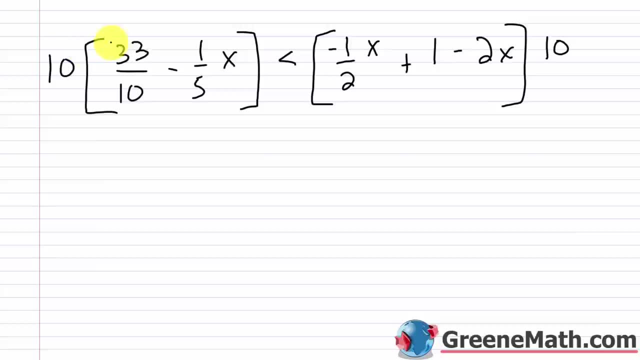 Close your brackets, And this is multiplied by 10 as well. So 10 times 33 over 10.. The 10s would cancel and you just have 33.. Then minus 10 times 1. fifth, 10 divided by 5 is 2.. 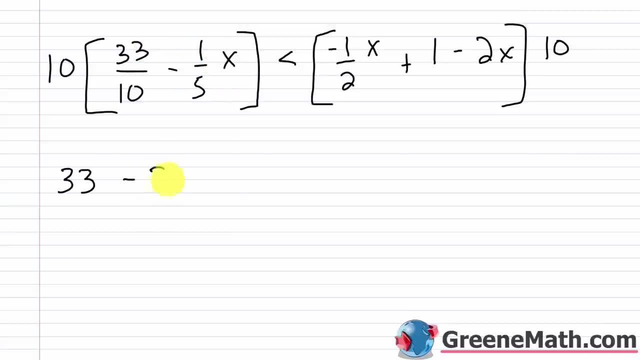 So then 2 times 1 is 2.. Then times x, So you just have minus 2 x And this is less than Over. here we have 10 times negative 1 half x. So the 10 would cancel the 2 and give me a 5.. 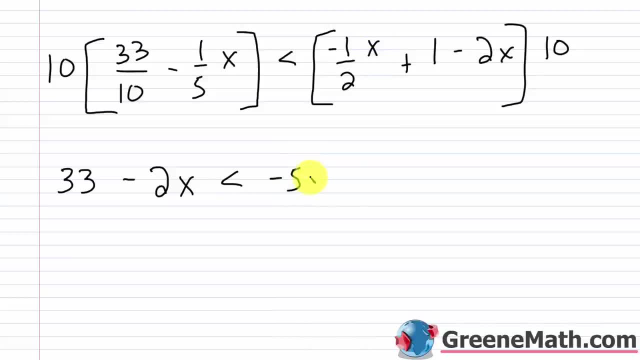 5 times negative, 1 is negative 5.. And then don't forget the x, So negative 5 x there. Then plus 10 times 1 is 10.. Then minus 10 times 2 x is 20 x. 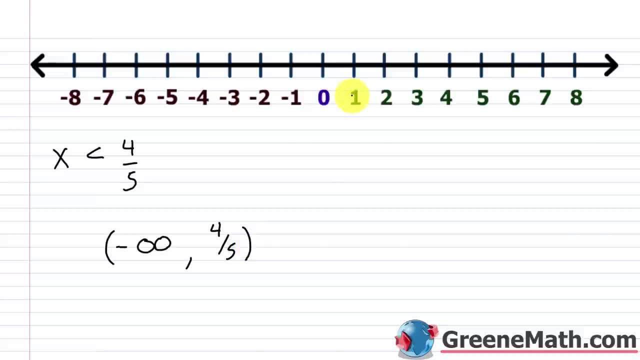 Now graphically we don't have a notch for 4 fifths. But let's say it's somewhere right there. 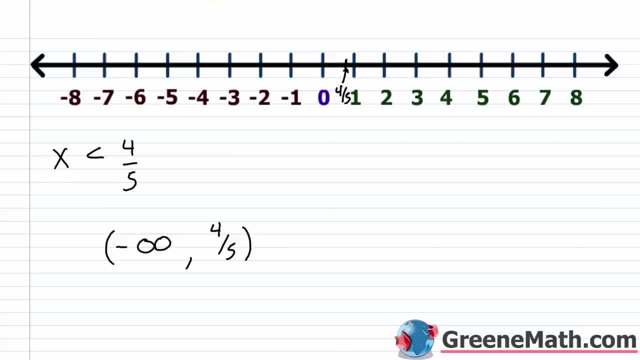 Let's say this is 4 fifths. I'll put the notch there. And so I'm going to use a parenthesis at 4 fifths. It's going to face to the left. And I'm going to shade everything to the left. Including this arrow right here. So that would be x is less than 4 fifths. 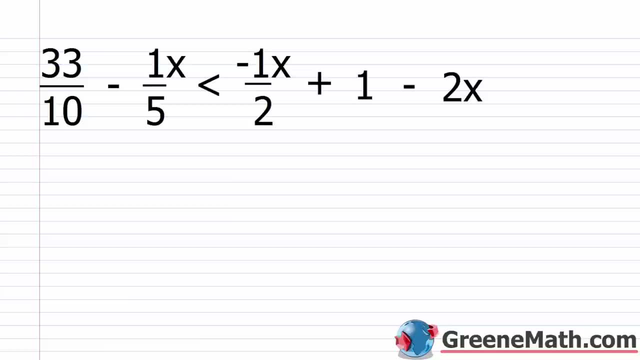 Alright, let's take a look at another one with some fractions. We have 33 tenths minus 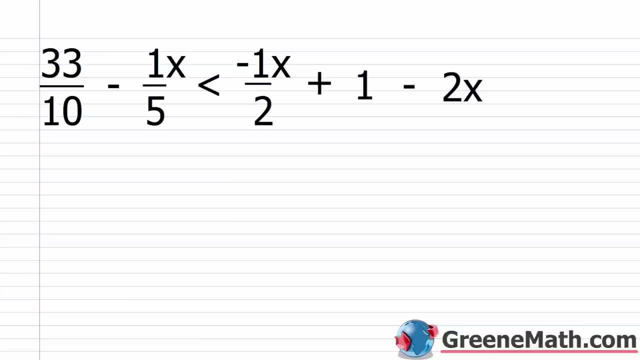 1 fifth x is less than negative 1 half x plus 1 minus 2 x. 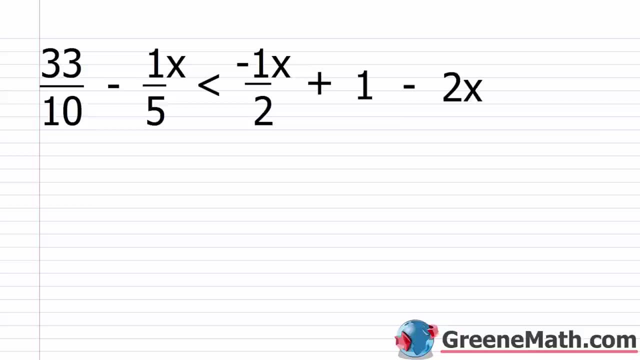 So the first thing I'm kind of looking at here is to clear the fractions the LCD is 10. 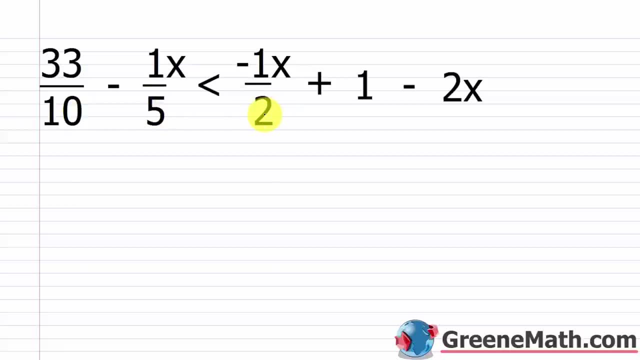 Alright, I have 5, I have 2, and I have 10. 5 times 2 is 10. So the LCD is 10. So let's multiply both sides of the inequality by 10. So I'd have 10 times, remember to use brackets, or again you could use parenthesis if you want. So 33 over 10 minus 1 fifth times x. 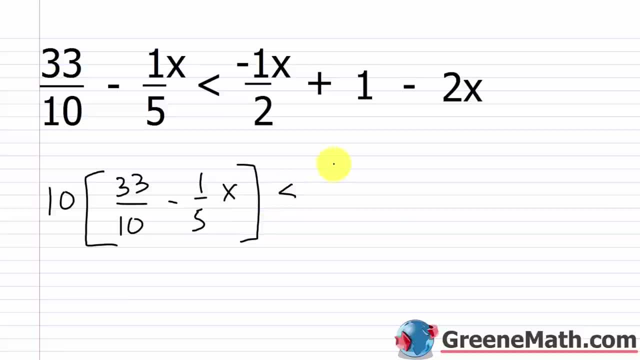 Close the brackets. And then this is less than. 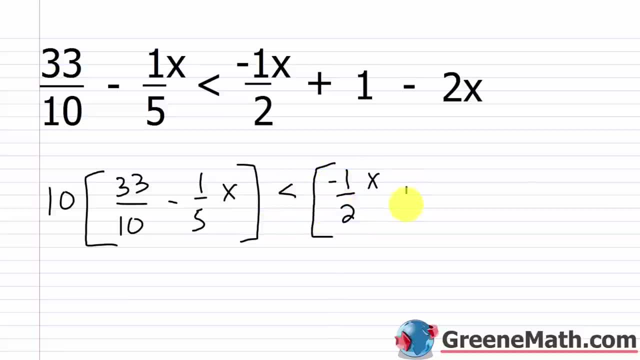 Open brackets. Negative 1 half times x plus 1 minus 2 x. Close your brackets. 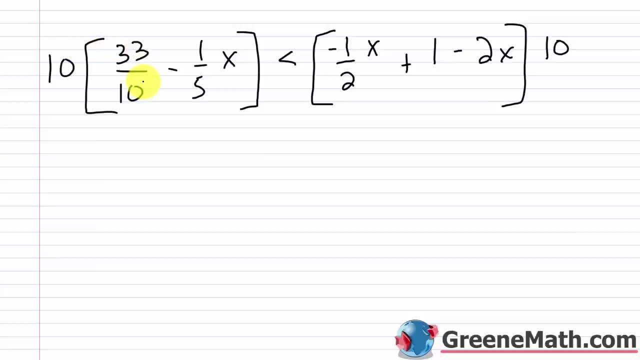 And this is multiplied by 10 as well. So 10 times 33 over 10. 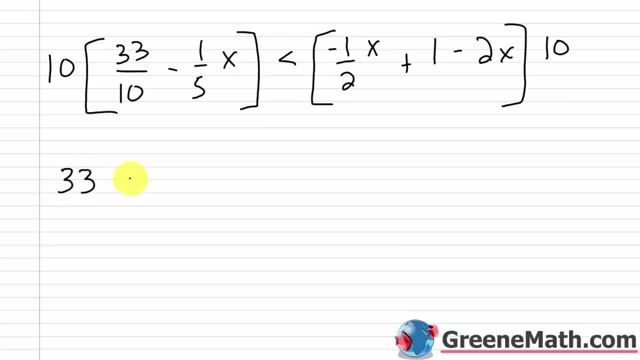 The 10's would cancel and you'd just have 33. 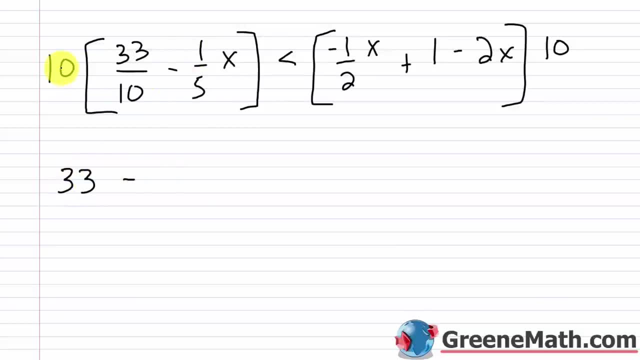 Then minus. 10 times 1 fifth. 10 divided by 5 is 2. So then 2 times 1 is 2. Then times x so you'd just have minus 2 x. 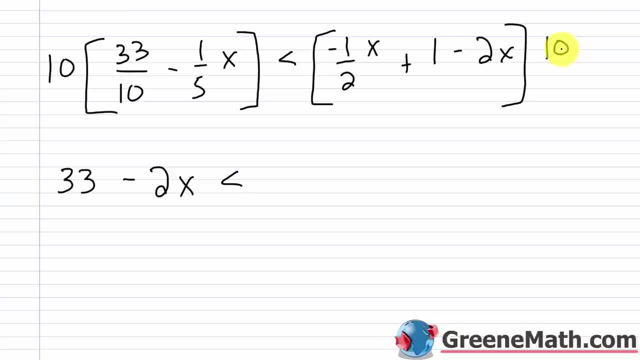 And this is less than. Over here we have 10 times 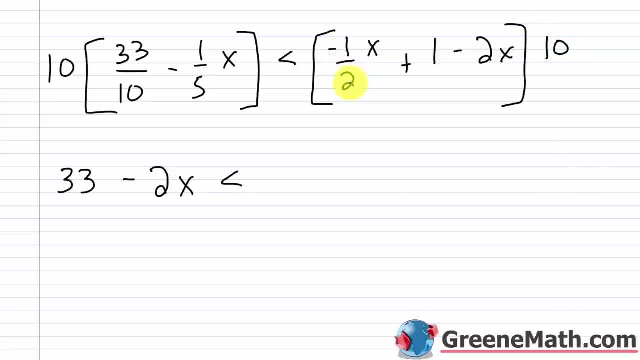 negative 1 half x. So the 10 would cancel with the 2 and give me a 5. 5 times negative 1 is negative 5. And then don't forget the x. So negative 5 x there. 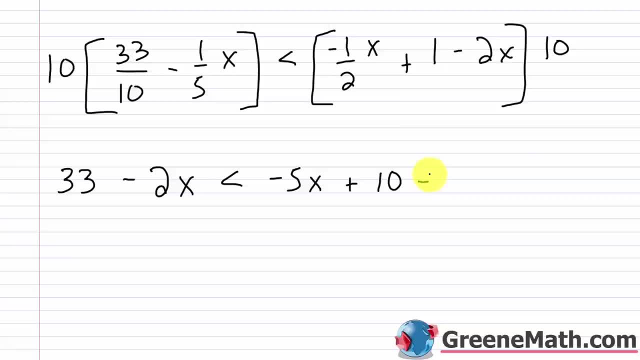 Then plus 10 times 1 is 10. Then minus 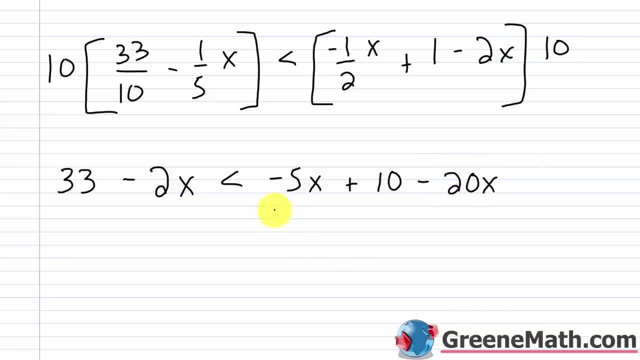 10 times 2 x is 20 x. So I can combine like terms on the right side here. 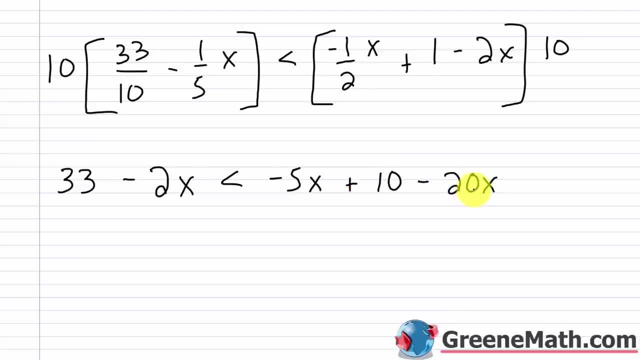 Negative 5 x minus 20 x is minus 25 x. So I'll put negative 25 x. Plus 10. 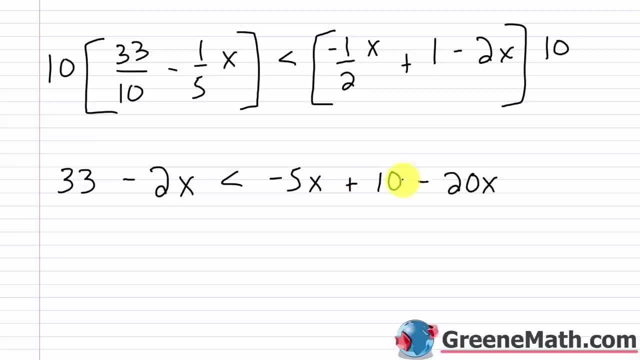 So I can combine like terms on the right side here: Negative 5 x minus 20 x is minus 25 x, So I'll put negative 25 x plus 10.. So over here nothing to combine. I'm just going to write negative 2 x out in front plus 33.. 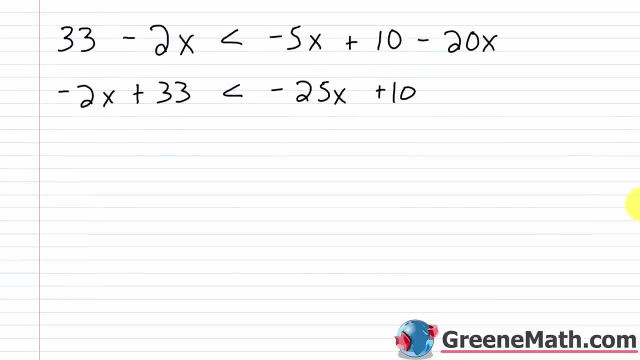 And now I want to get a variable, A variable term on one side of the inequality and a number on the other. So in order to do that, I'm going to add 25 x to both sides of the inequality. That's gone. And negative. 2 x plus 25 x would be 23 x. 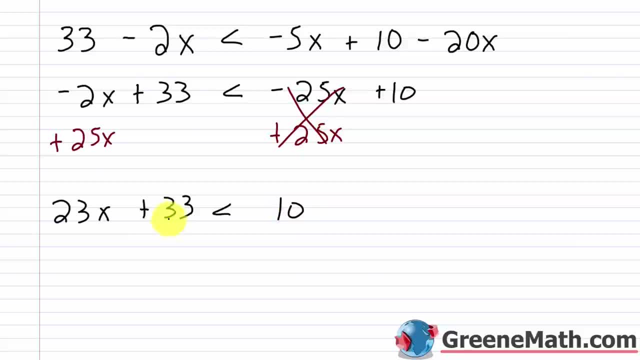 So then plus 33 is less than 10.. I'm going to move this over here. I'm going to simply subtract 33 from both sides of the inequality. So this is gone, And I'm going to end up with 23. x is less than 10 minus 33 is negative 23.. 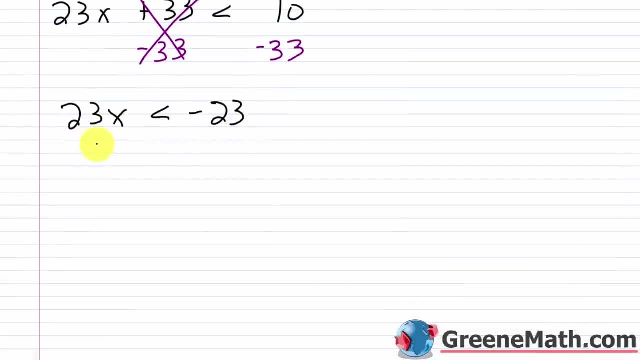 So, as a final step, I'm going to divide both sides of the inequality by 23.. Which is the coefficient of x. So divide this by 23 and this by 23.. And I'm going to get x is less than negative 1.. 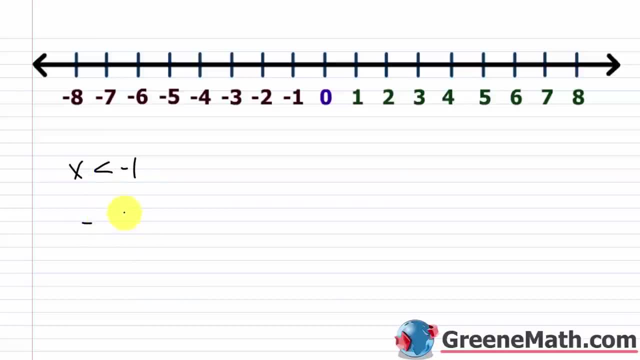 All right. so an interval notation Again, the smallest possible value. if you're dealing with the less than, It's less than negative 1.. So this would continue to the left Forever and ever and ever. So we write negative infinity here And we always use a parenthesis with infinity or negative infinity. 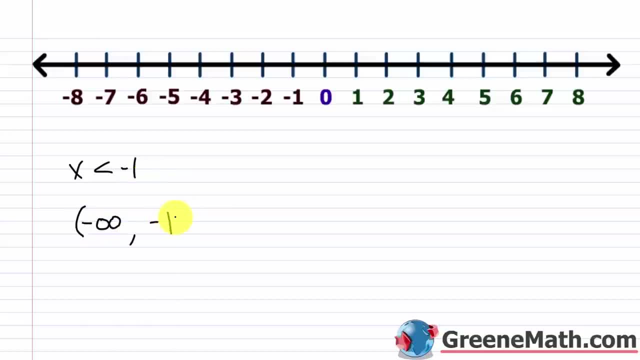 And then comma. for the largest possible value. we put negative 1. And again, that's not included. So we put a parenthesis there. to show that Now graphically, I'm just going to put a parenthesis at negative 1.. Facing to the left. 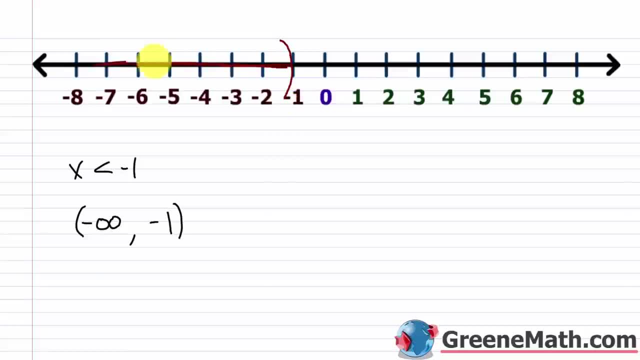 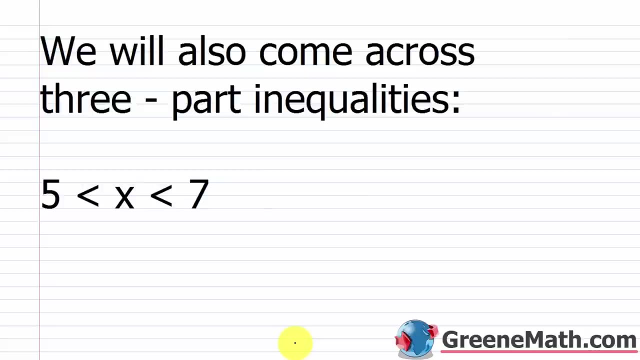 Facing towards the solution. And then I'm going to shade everything to the left, Including that arrow, to say, hey, negative 1 is not included, So I got the parenthesis there, But everything to the left of that would be. So another thing we're going to come across will be three part inequalities. 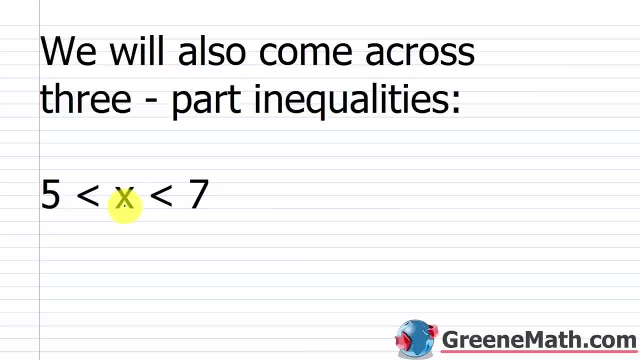 So you see here we have: 5 is less than x and x is less than 7.. Where you could say x is greater than 5 and x is less than 7.. What's important to note here is that both conditions have to be true. 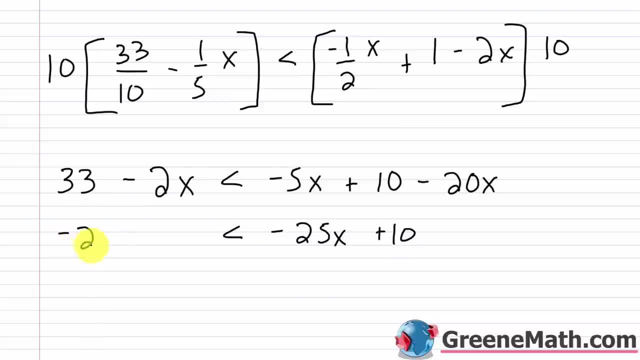 So over here nothing to combine. I'm just going to write negative 2 x out in front. Plus 33. 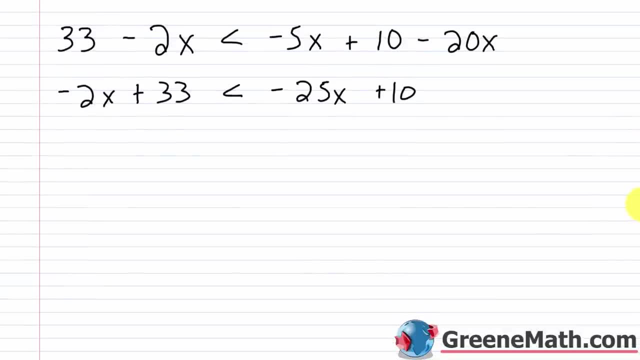 And now I want to get a 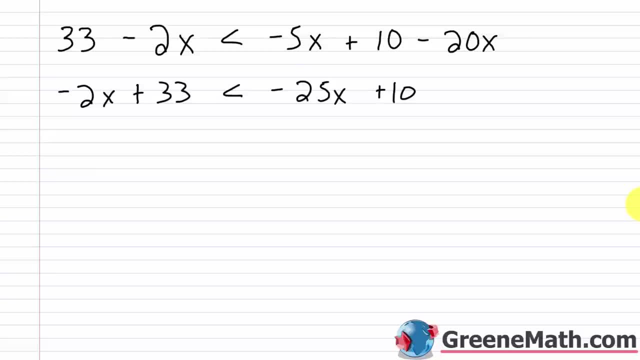 variable term on one side of the inequality and a number on the other. 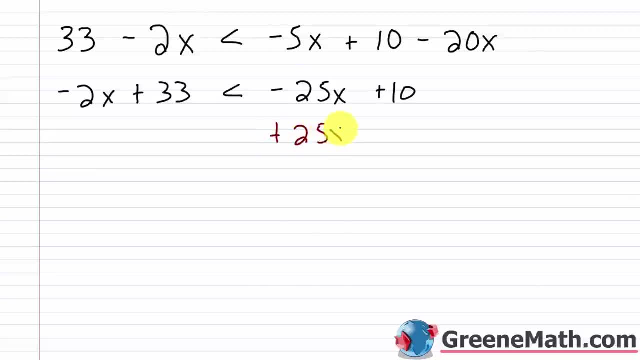 So in order to do that I'm going to add 25 x to both sides of the inequality. That's gone. 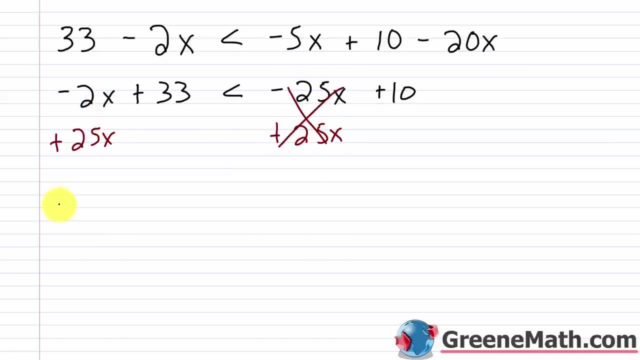 And negative 2 x plus 25 x would be 23 x. 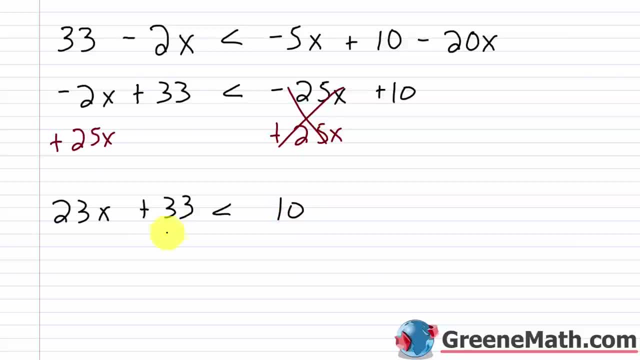 So then plus 33 is less than 10. I'm going to move this over here. I'm going to simply subtract 33 from both sides of the inequality. So this is gone. 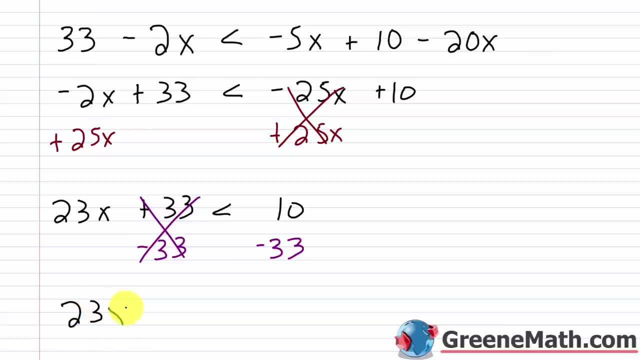 And I'm going to end up with 23 x is less than 10 minus 33 is negative 23. 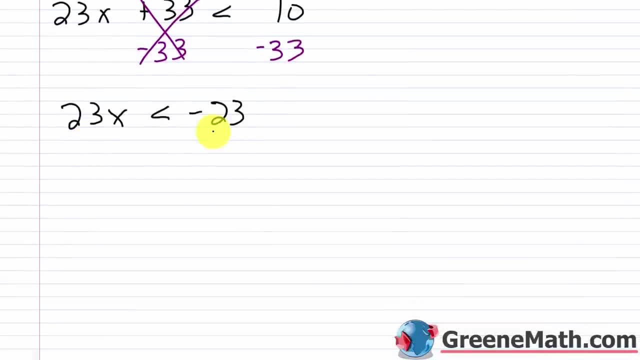 So as a final step I'm going to divide both sides of the inequality by 23. Which is the coefficient of x. So divide this by 23 and this by 23. And I'm going to get x is less than negative 1. 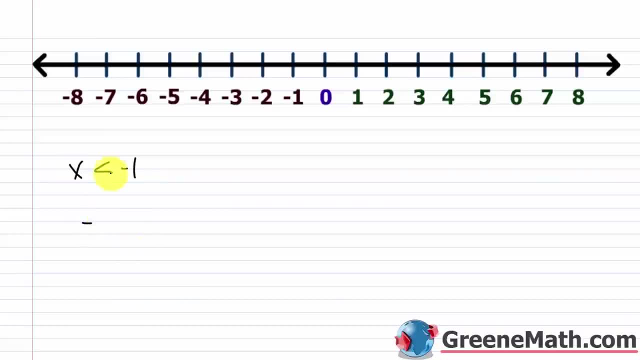 Alright, so an interval notation again, the smallest possible value if you're dealing with a less than it's less than negative 1. So this would continue to the left forever and ever and ever. So we write negative infinity here. And we always use a parenthesis with infinity or negative infinity. And then comma for the largest possible value we put negative 1. And again that's not included. So we put a parenthesis there to show that. 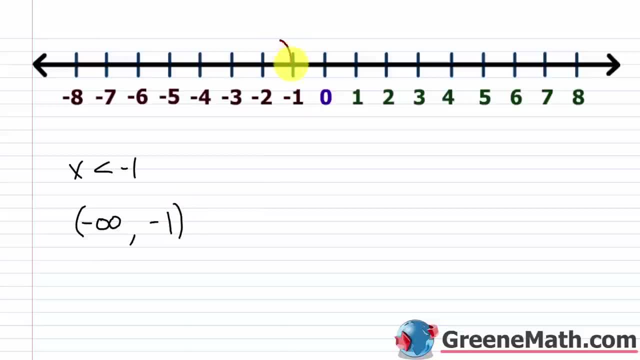 Now graphically I'm just going to put a parenthesis at negative 1 facing to the left, facing towards the solution. And then I'm going to shade everything to the left including that arrow to say hey, negative 1 is not included so I got the parenthesis there. But everything to the left of that would be. 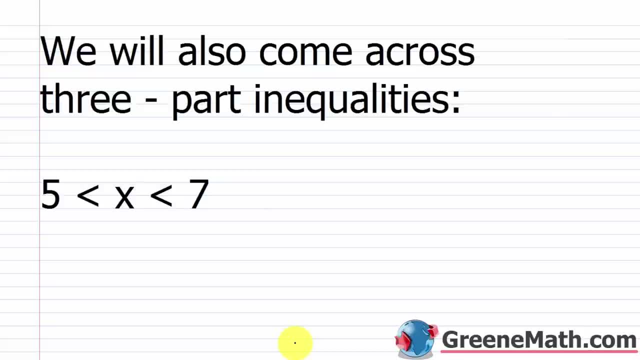 So another thing we're going to come across will be three part inequalities. So you see here we have 5 is less than x and x is less than 7. Or you could say x is greater than 5 and x is less than 7. What's important to note here is that both conditions have to be true. 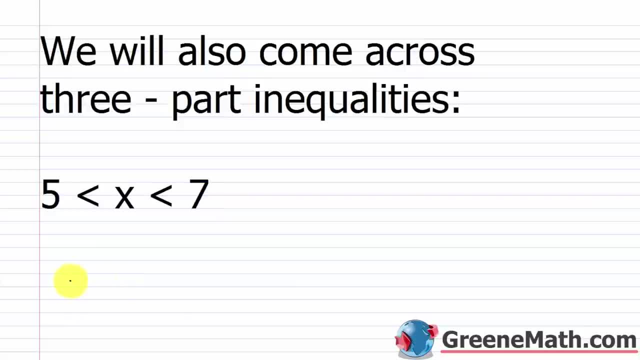 So in other words you can kind of think of these as separate problems. I can kind of think of this as x is greater than 5. 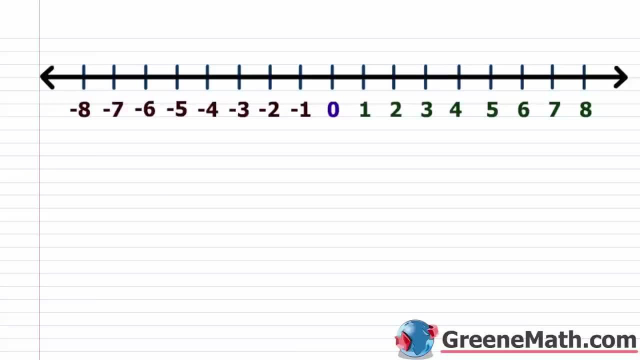 So if I was to graph that x is greater than 5 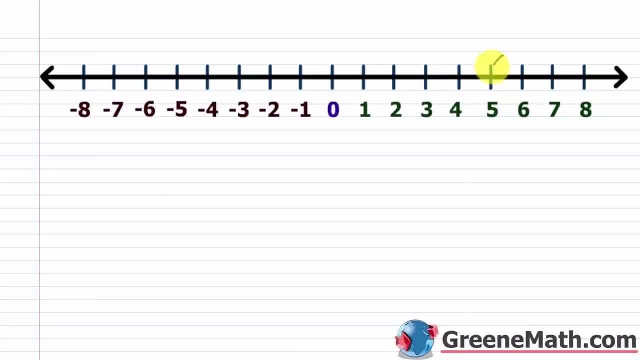 I would think about what? I would think about putting a parenthesis here and I would graph everything to the right of 5. 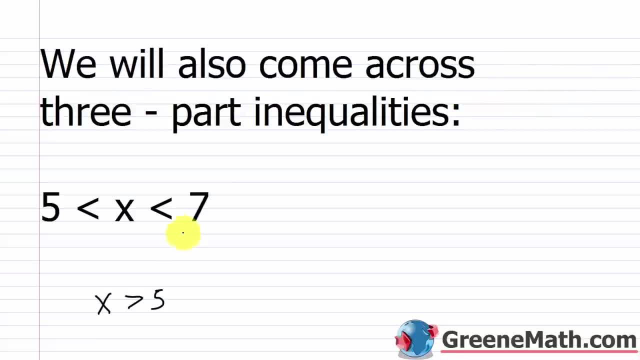 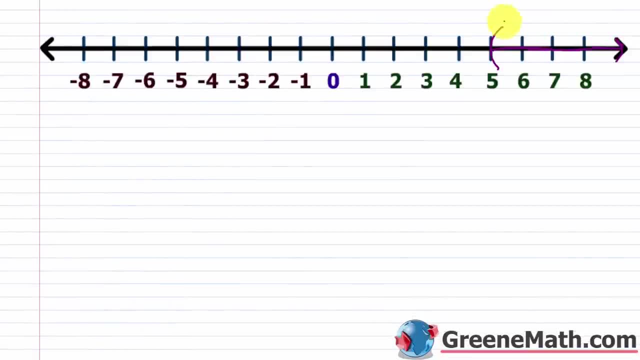 And then for the other part of this problem x is less than 7. Now if I graphed that I would put a parenthesis at 7 and I would graph everything to the left. Everything to the left. 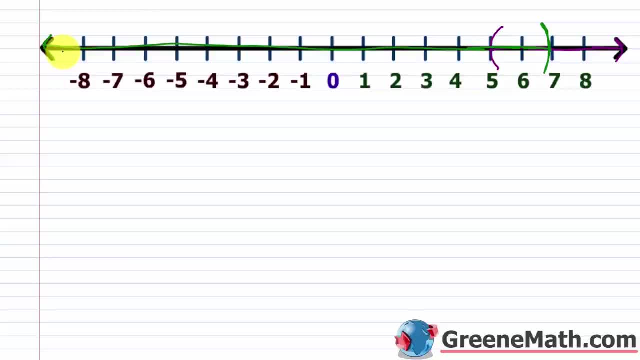 Now when we have a three part inequality we're kind of combining the two and saying hey I only want the section that solves both. So if we look at what's shaded by both and it's kind of hard to tell but it's going to be this area between 5 and 7. 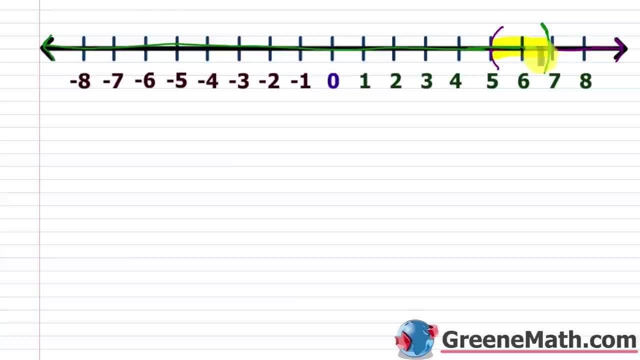 So x is not included and 7 is not included. But anything between those two would be included. 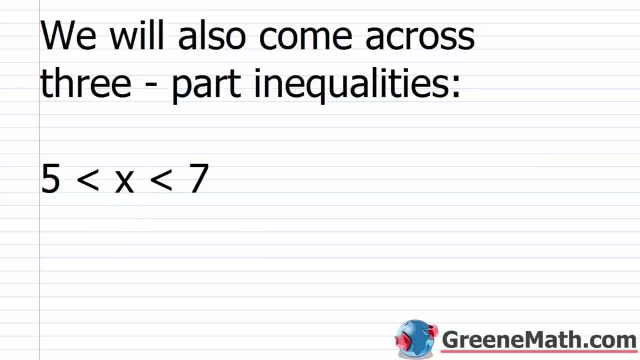 If you think about it it should make sense to you. Let me kind of erase this. 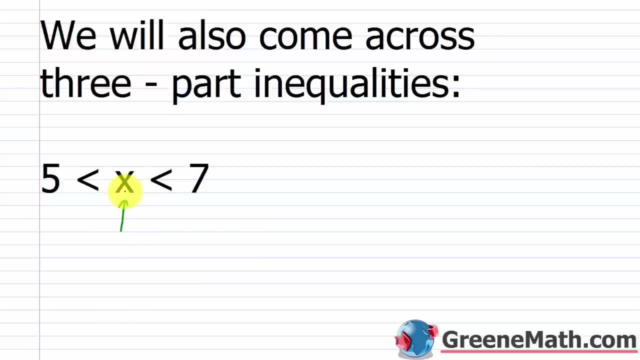 x can be any number that satisfies both conditions. So if I plug in something between 5 and 7 like 6 6 is greater than 5 and 6 is also less than 7 so that works out. 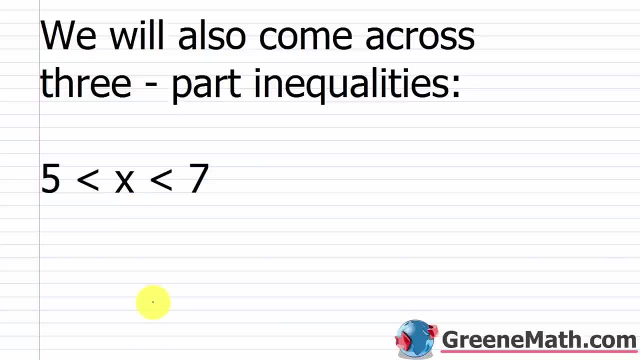 If I plug in something that is outside of the solution region let's say I plug in x is 0 well 0 is not greater than 5. It's less than 7 but it's not greater than 5. So it doesn't satisfy the inequality because one part fails and it's got to be a solution to both. 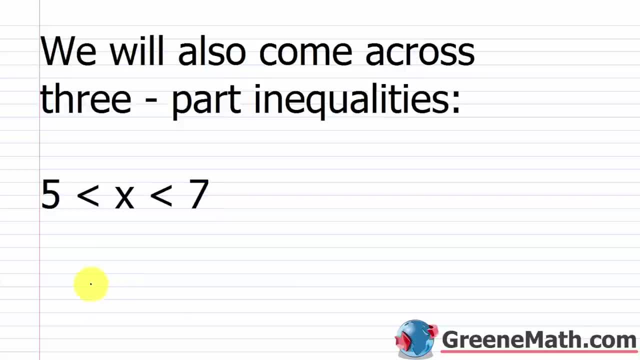 So, in other words, you can kind of think of these as separate problems. I can kind of think of this as x is greater Than 5.. So if I was to graph that x is greater than 5. I would think about what. 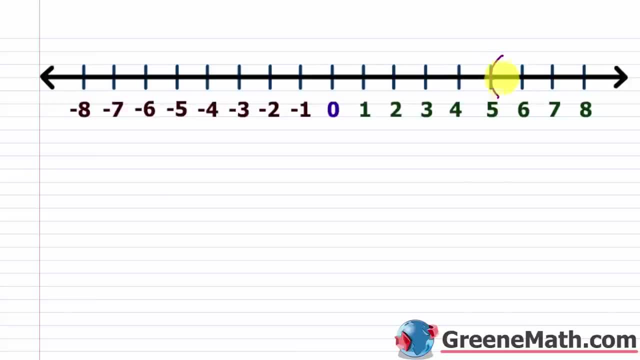 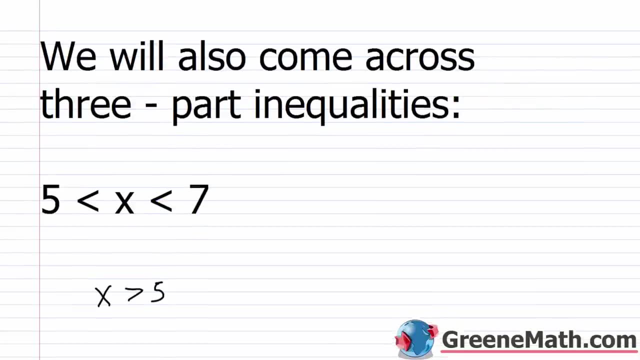 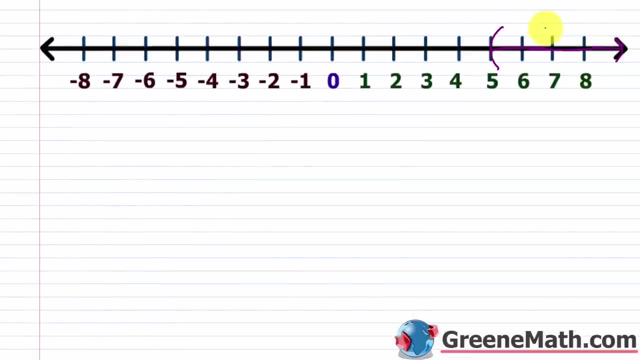 I would think about putting a parenthesis here And I would graph everything to the right of 5. And then, for the other part of this problem, x is less than 7.. So x is less than 7.. Now, if I graphed that, I would put a parenthesis at 7.. 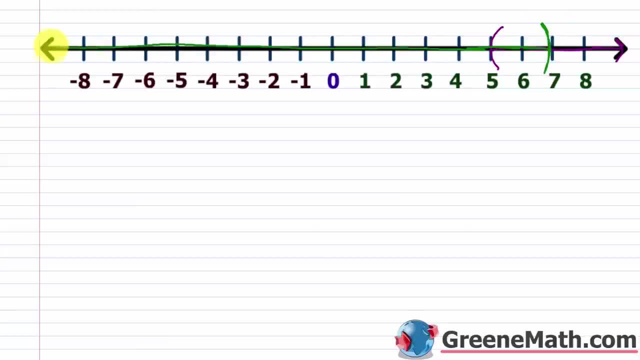 And I would graph everything to the left, Everything to the left. Now, when we have a three part inequality, we're kind of combining the two and saying, Hey, I only want the section that solves both. So if we look at what's shaded by both and it's kind of hard to tell. 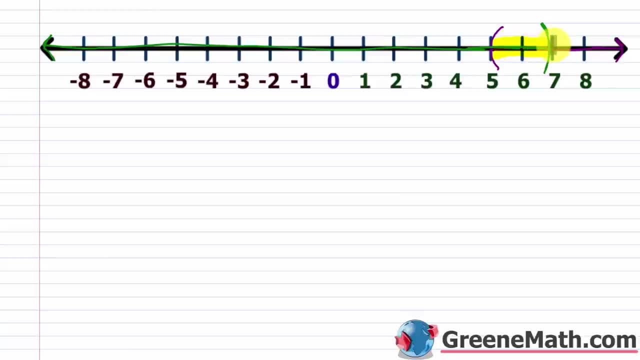 But it's going to be this area between 5 and 7.. 5 is not included and 7 is not included, But anything between those two would be included. If you think about it, it should make sense to you. Let me kind of erase this. 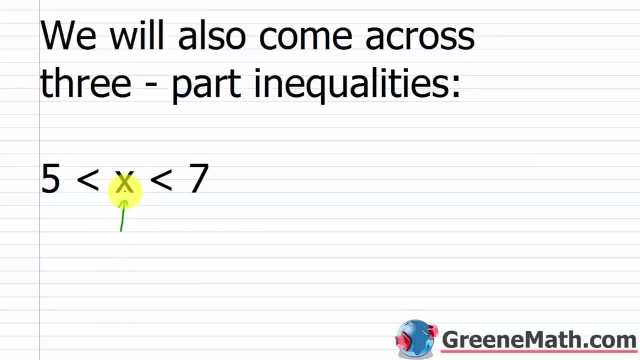 x can be any number that satisfies both conditions. So if I plug in something between 5 and 7, like 6. 6 is greater than 5. And 6 is also less than 7.. So that works out If I plug in something that is outside of the solution region for one of them. 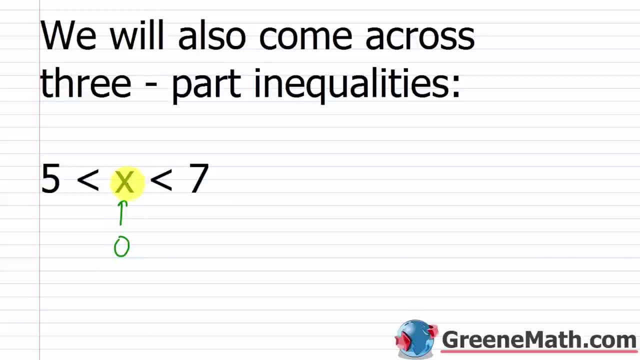 Let's say I plug in- x is 0. Well, 0 is not greater than 5. It's less than 7, but it's not greater than 5.. So it doesn't satisfy The inequality because one part fails and it's got to be a solution to both. 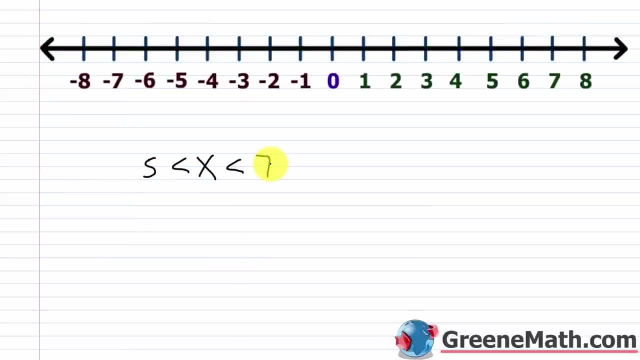 All right, so let's graph this again from scratch. You're going to start out at your smallest value, And in this case, it's going to be us starting at 5- with a parenthesis, Because 5 is not included- And then we're going to look at our largest value. 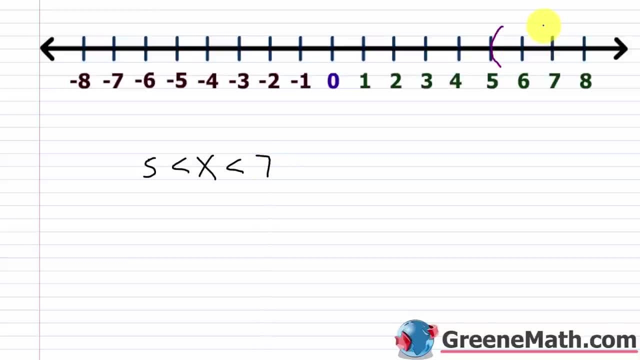 And that's going to be us going to 7.. And putting a parenthesis, because 7 is not included And we shade all the area between, All the area between. So anywhere in there is a solution. I know we think about 6 because it's a nice neat whole number. 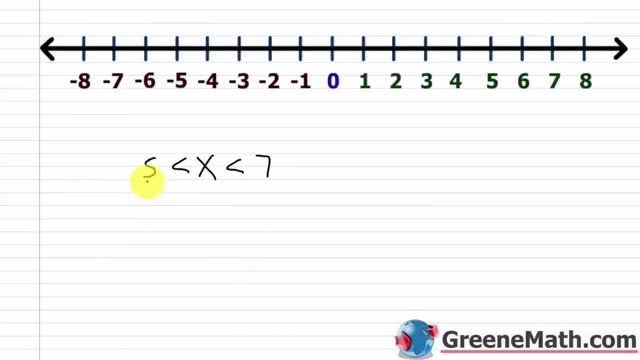 So let's graph this again from scratch. You're going to start out at your smallest value and in this case it's going to be us starting at 5 with a parenthesis because 5 is not included and then we're going to look at our largest value and that's going to be us going to 7 and putting a parenthesis because 7 is not included and we shade all the area between. 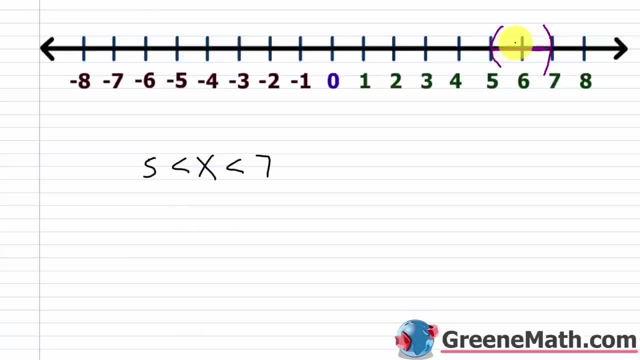 All the area between. So anywhere in there is a solution. 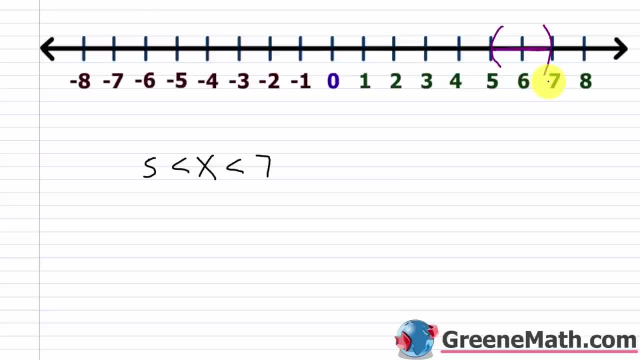 I know we think about 6 because it's a nice neat whole number 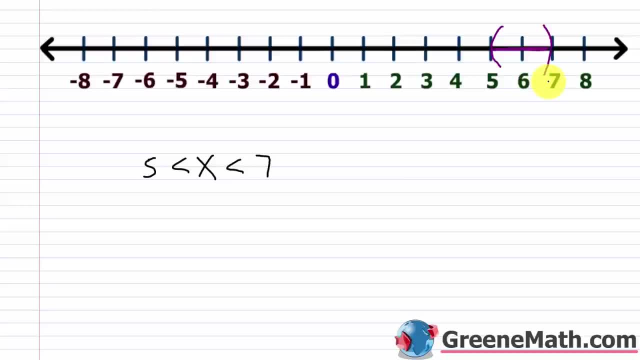 but really anything between 5 and 7 so 5.12228 would be a solution because that's larger than 5 and less than 7. 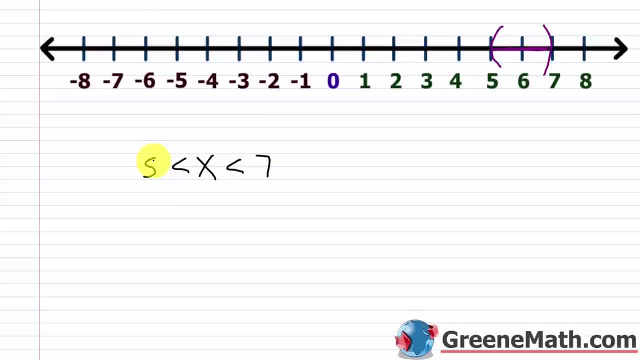 Now in interval notation it kind of follows a similar pattern. 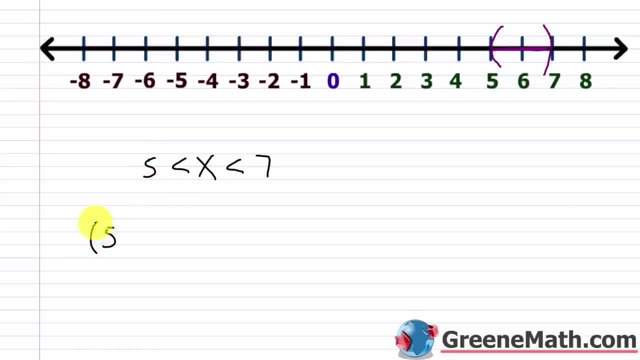 For our smallest number we'd put 5 and a parenthesis next to it to say 5 is not included 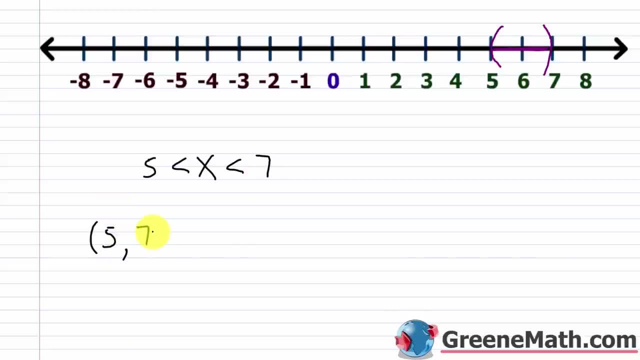 then comma we'd put 7 for the largest and a parenthesis to say 7 is not included. 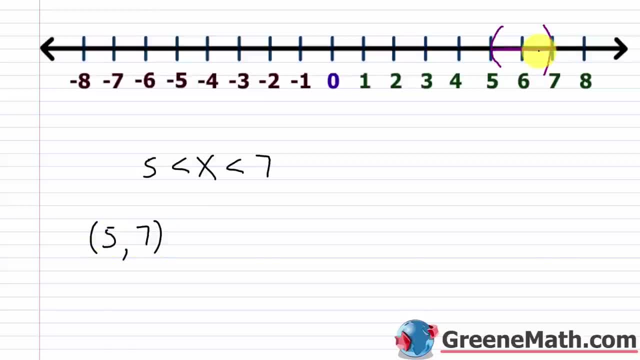 So this is your interval notation and here is your graph. So to solve a 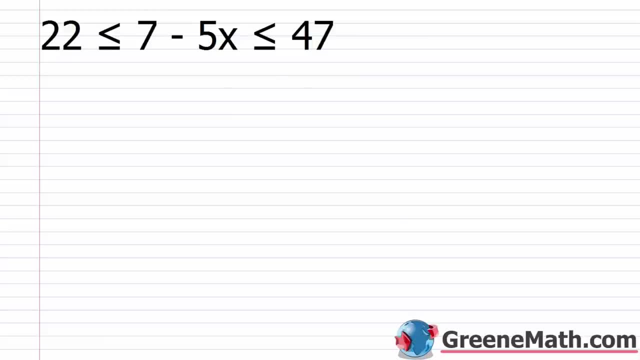 three part inequality is no more difficult than solving a regular inequality. 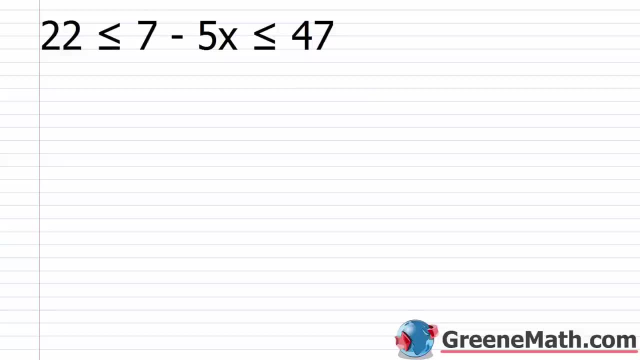 Now you can do it two ways. And the most popular way, the easiest way is kind of to do the same thing to each part. So let me kind of show you that way first. So I'm trying to isolate the variable 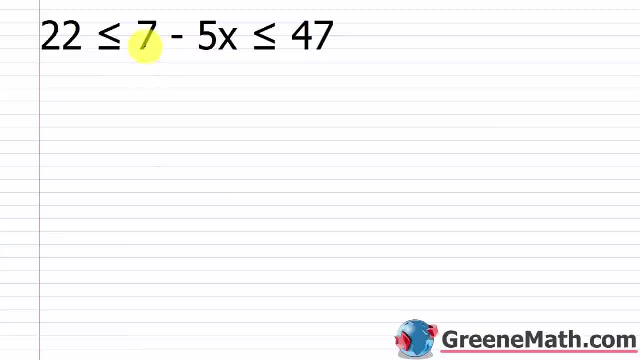 in the middle. And in order to do that I just think about okay I have 7 here. I'm going to subtract away 7 from each part. And this is the tricky thing because we're used to just doing it to two sides. 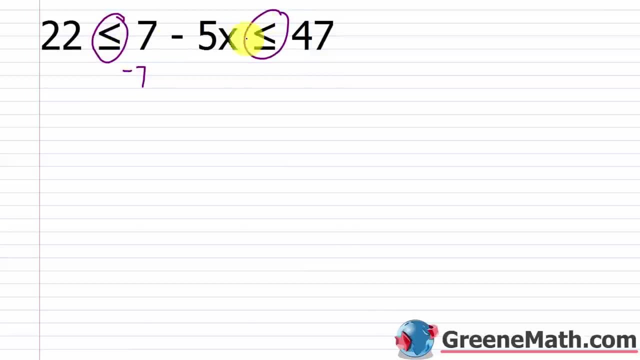 Now I have this here and this here. So everywhere I see that I've got to subtract away from that part. So subtract away 7 from here, here, and here. Right? All three parts. So this will cancel. And 22 minus 7 is 15. So I have 15 is less than or equal to negative 5x which is less than or equal to 47 minus 7 is 40. 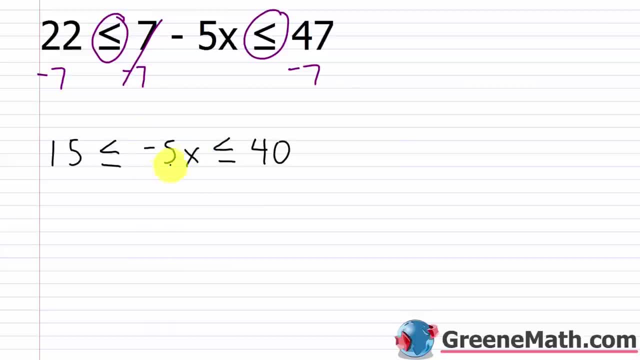 Now to isolate x in the middle I have this negative 5. 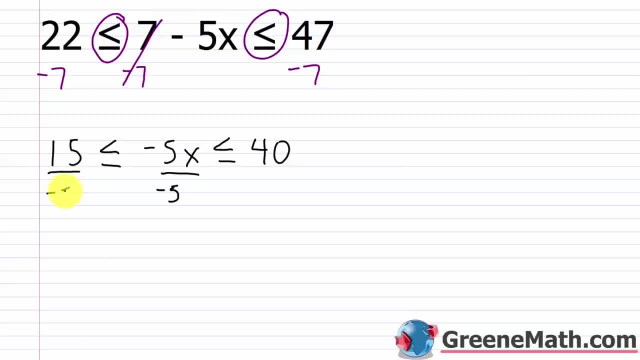 I'm going to divide each part by negative 5. Each part by negative 5. 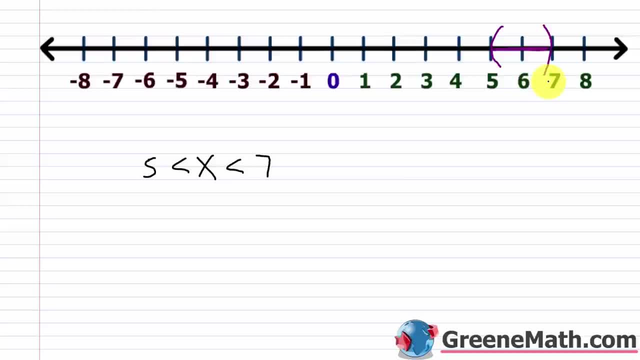 But really anything between 5 and 7.. So 5.122228 would be a solution, right, Because that's larger than 5 and less than 7.. Now in interval notation it kind of follows a similar pattern. For our smallest number we'd put 5 and a parenthesis next to it to say 5 is not included. 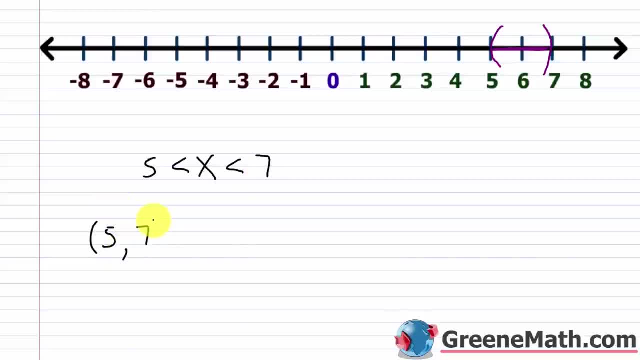 Then comma, we'd put 7 for the largest And a parenthesis to say 7 is not included. So this is your interval notation And here is your graph. So to solve a three part inequality is no more difficult than solving a regular inequality. 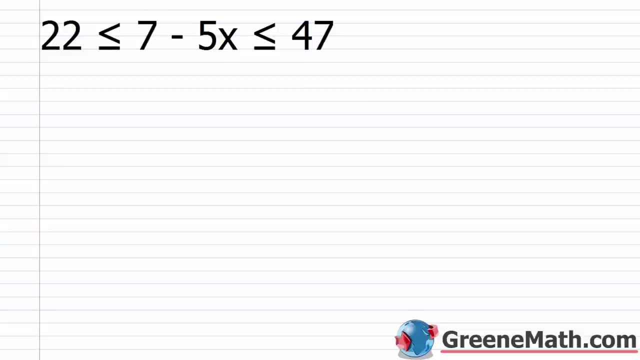 Now you can do it two ways, And the most popular way, the easiest way, is kind of to do the same thing to each part. So let me kind of show you that way first. So I'm trying to isolate the variable in the middle. 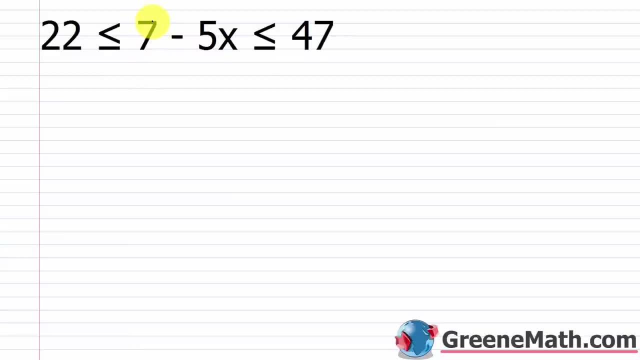 And in order to do that, I just think about: okay, I have 7 here, I'm going to subtract away 7 from each part, And this is the tricky thing, because we're used to just doing it to two sides. Now I have this here and this here. 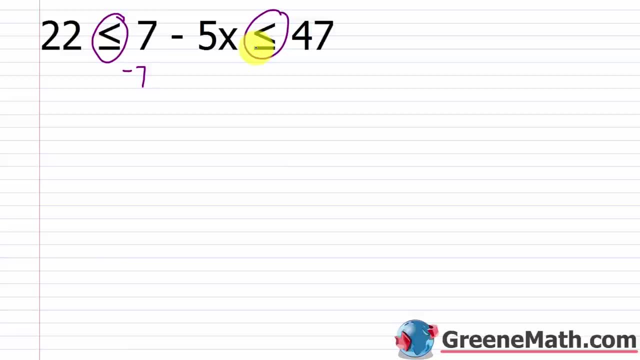 So everywhere I see that I've got to subtract away from that part. So subtract away 7 from here, here and here, right, All three parts. So this will cancel, And 22 minus 7 is 15.. So I have 15 is less than or equal to negative 5x. 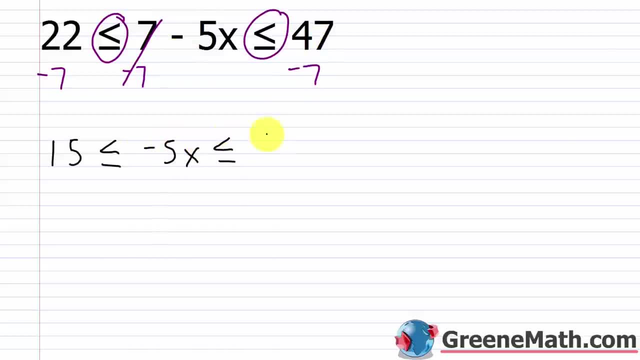 Which is less than or equal to, 47 minus 7 is 40. Now to isolate x in the middle, I have this negative 5.. I'm going to divide each part by negative 5.. Each part by negative 5.. Each part by negative 5.. 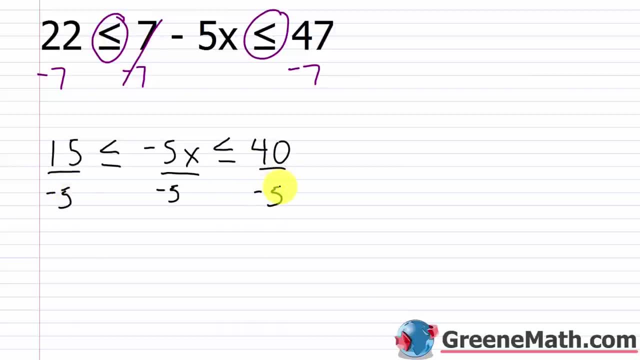 Now remember, when I divide by a negative, I've got to flip. And I've got two signs here. I've got to flip both of them. So this is going to flip this way And this is going to flip this way as well. 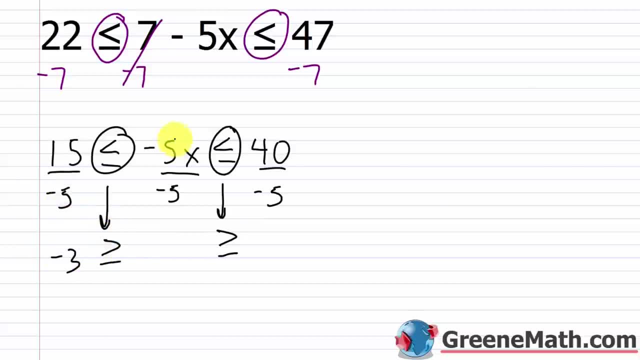 So 15 divided by negative, 5 is negative 3.. Negative 5 divided by negative 5 is 1.. So this is just x 40 divided by negative, 5 is negative 8.. Now I'm going to rewrite this. 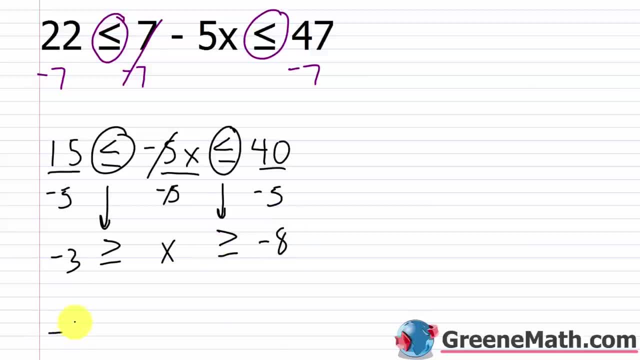 I want my smallest number on the left, So I'm going to put negative 8.. And it's less than or equal to x, So I'm going to put less than or equal to x. And then I'm going to put x is less than or equal to negative 3.. 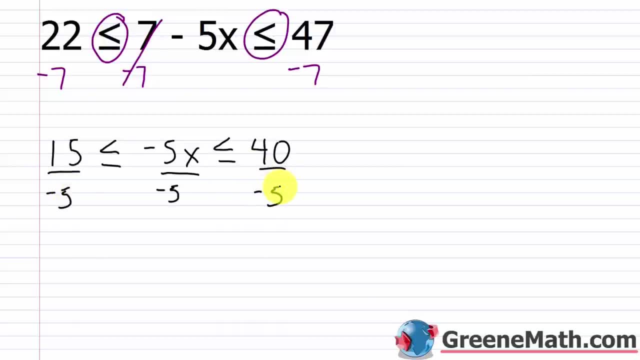 Each part by negative 5. Now remember 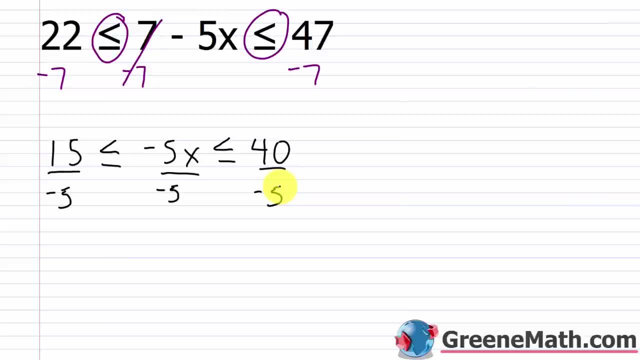 when I divide by a negative I've got a flip. And I've got two signs here I've got to flip both of them. 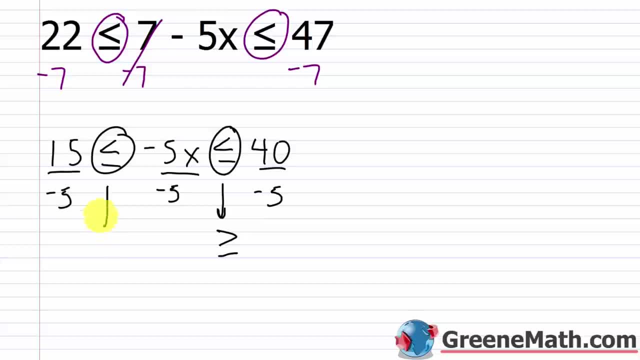 So this is going to flip this way. And this is going to flip this way as well. 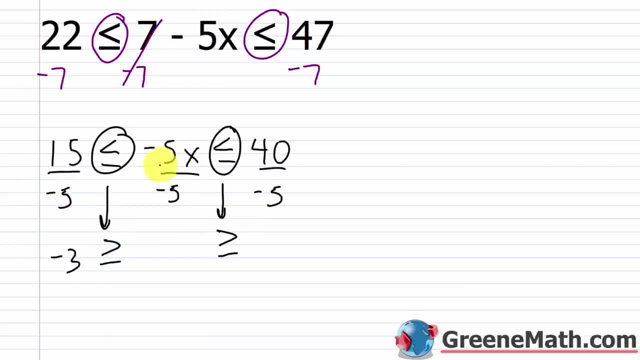 So 15 divided by negative 5 is negative 3. Negative 5 divided by negative 5 is 1. So this is just x. 40 divided by negative 5 is 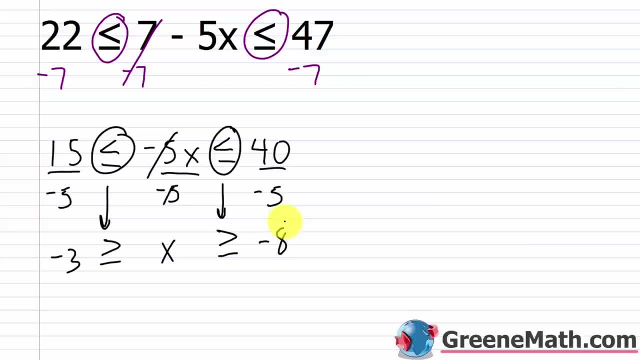 negative 8. Now I'm going to rewrite this. I want my smallest number on the left. So I'm going to put negative 8. And it's less than or equal to x. So I'm going to put less than or equal to x. 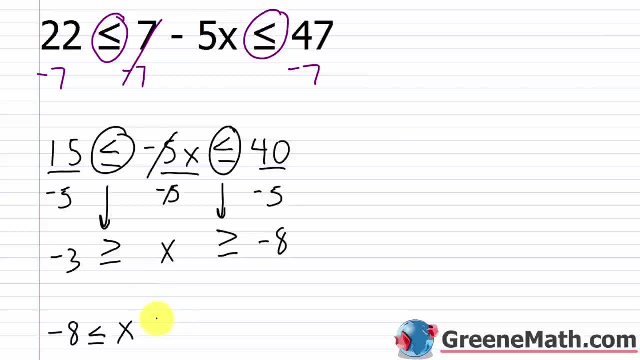 And then I'm going to put x is less than or equal to negative 3. So now this runs in the order of the number line. And that's my solution. 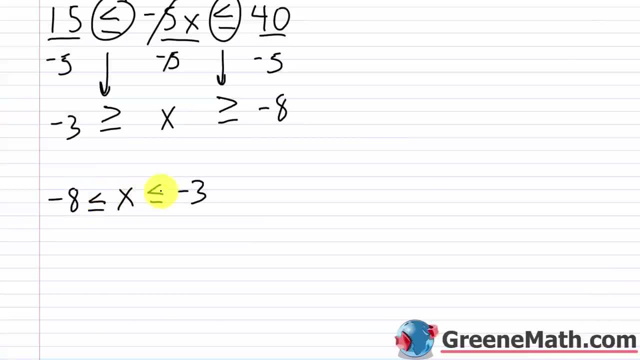 x is greater than or equal to negative 8 and it's also less than or equal to negative 3. If I find negative 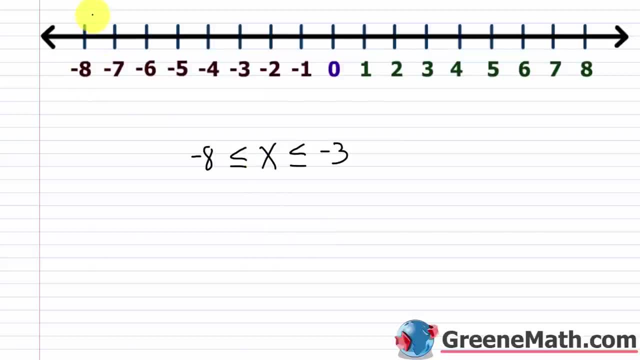 8 on the number line, that's right here. I would put a bracket there because negative 8 is included. 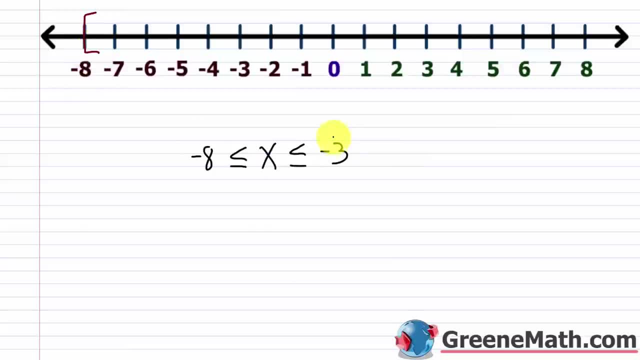 So that's the smallest value that x can take on. Negative 3 is the largest value that x can take on. So I put my bracket there. 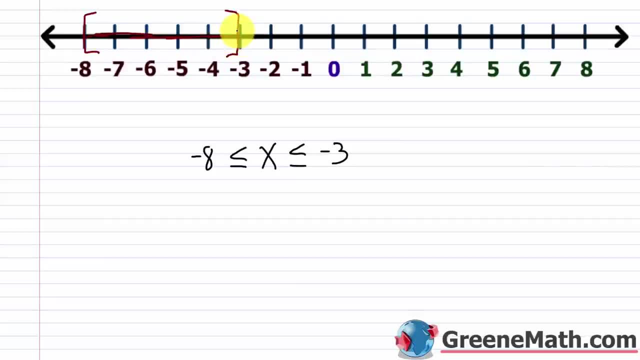 And shade everything in between. So I'm saying that x can be negative 8 and larger up to and including negative 3. Anywhere in those values would work. If I picked 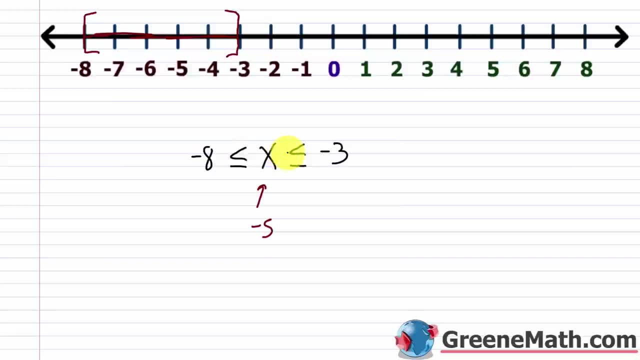 negative 5. Well negative 5 is larger than negative 8 and it's smaller than negative 3. So that works. 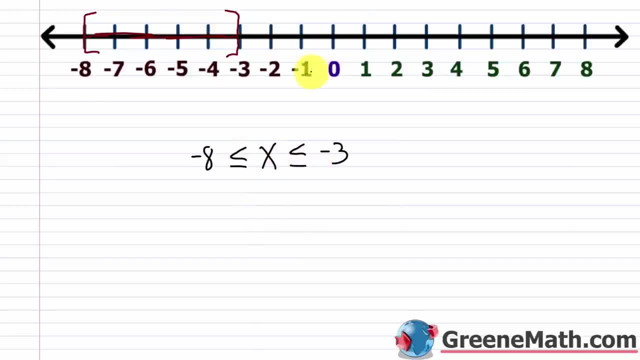 If I picked something outside of this range in the non-solution region, let's say 0. Plug that in. 0 is larger than negative 8 but it's not smaller than negative 3. So that doesn't work. So it's got to be something in this range of values. 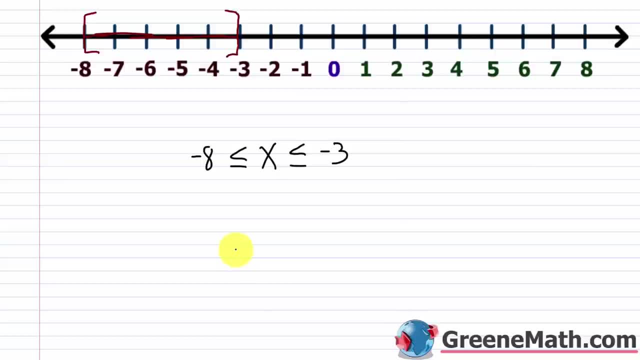 Now for my interval notation, I would put negative 8 as the smallest possible value. And I'd use a bracket there because negative 8 is included. And then I'd put negative 3 as my largest 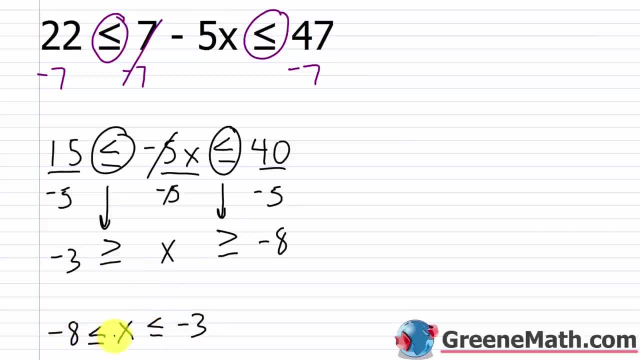 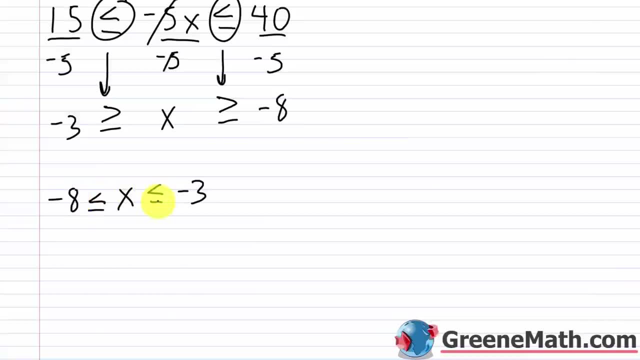 So less than or equal to negative 3.. So now this runs in the order of the number line, And that's my solution. x is greater than or equal to negative 8.. And it's also less than or equal to negative 3.. 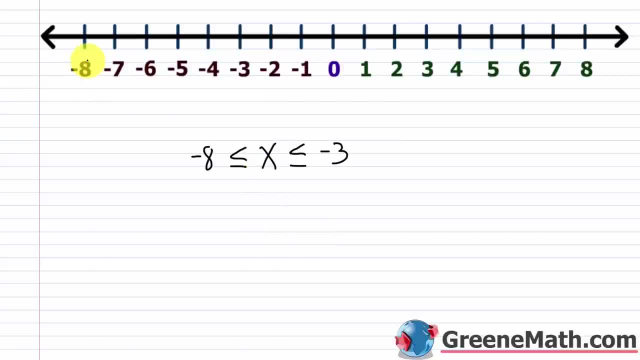 If I find negative 8 on the number line, that's right here. I would put a bracket there because negative 8 is included. So that's the smallest value that x can take on. Negative 3 is the largest value that x can take on. 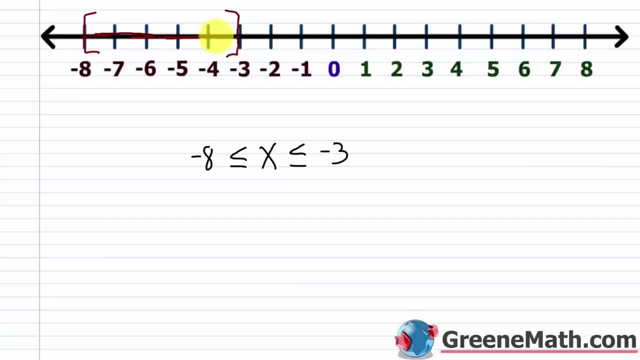 So I put my bracket there And shade everything in between. So I'm saying that x can be negative 8 and larger, up to and including negative 3. Anywhere in those values Would work If I picked negative 5.. Well, negative 5 is larger than negative 8.. 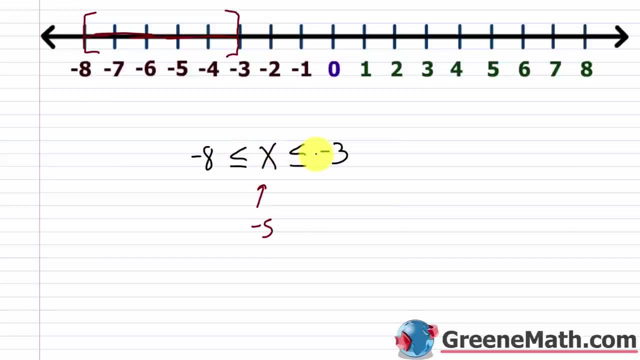 And it's smaller than negative 3.. So that works. If I picked something outside of this range In the non-solution region, Let's say 0.. Plug that in. 0 is larger than negative 8. But it's not smaller than negative 3.. 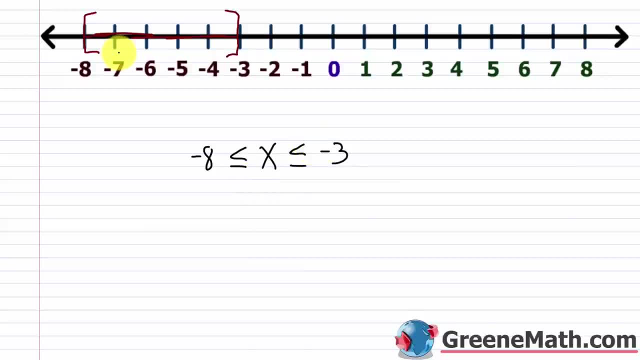 So that doesn't work Right. So it's got to be something in this range of values. Now for my interval notation. I would put negative 8 as the smallest possible value And I'd use a bracket there, Right, Because negative 8 is included. 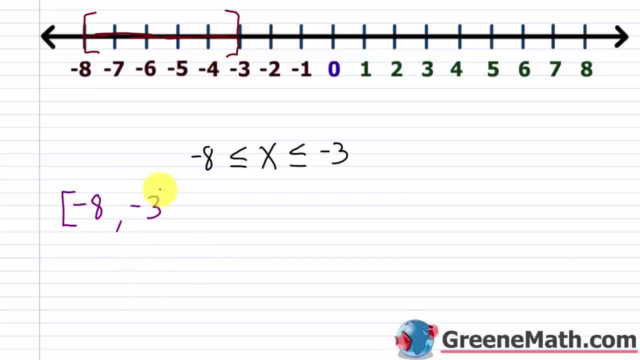 And then I'd put negative 3 as my largest possible value, And then a bracket next to it Again, because negative 3 is included. All right, So let's look at one more problem. So we have that negative 5 minus 12x is greater than or equal to negative 5.. 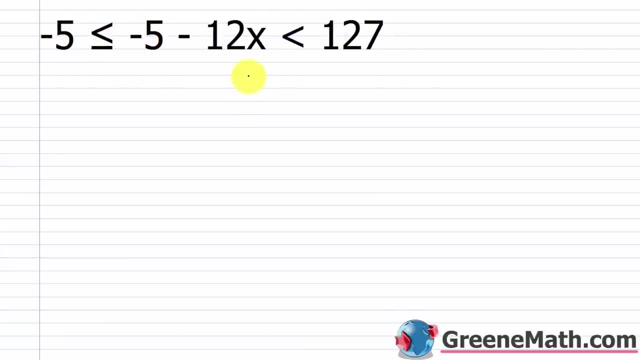 And less than 127.. So my goal is to isolate the variable x in the middle here. So I'm going to add 5 to each part. Remember, you got to do it to each part, But I'm going to add 5 to each part. 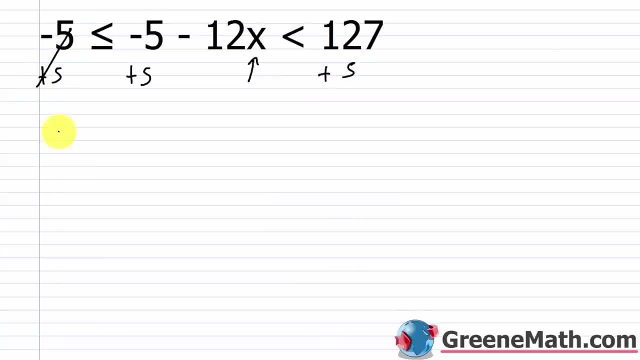 So that's going to cancel and be 0.. Make sure you write 0 there. You don't have anything else over there. So this is less than or equal to, And then this is going to cancel. I'll just have negative 12x in the middle. 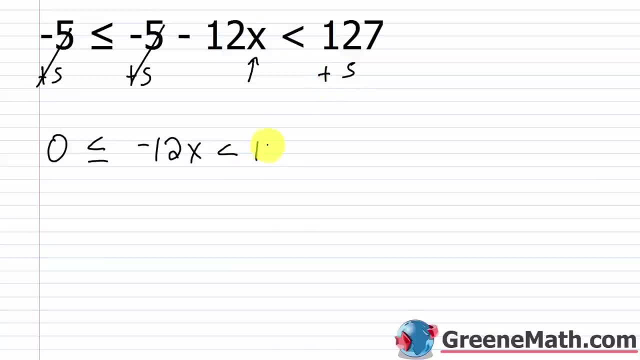 And then, as less than We have, 127 plus 5. That's 132.. And now I'm going to divide each part by negative 12.. Again, because I'm dividing by a negative, I've got to flip all the signs. 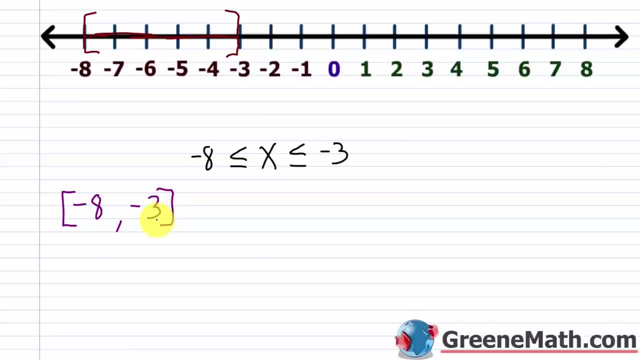 possible value. And then a bracket next to it again because negative 3 is 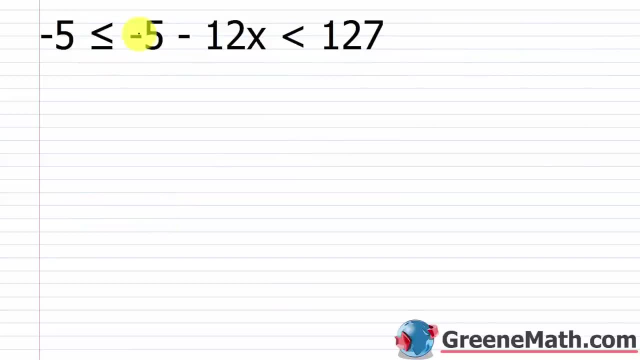 included. Alright so let's look at one more problem. So we have that negative 5 minus 12x is greater than or equal to negative 5 and less than 127. So my goal is to isolate the variable x in the middle here. 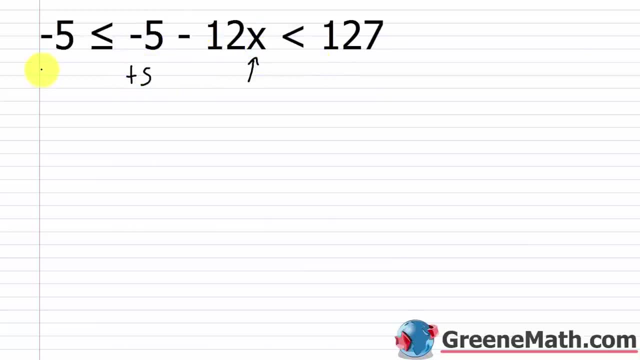 So I'm going to add 5 to each part. Remember you've got to do it to each part. 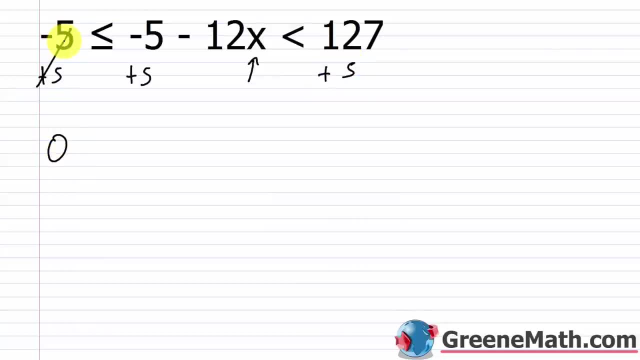 So that's going to cancel and be 0. Make sure you write 0 there. You don't have anything else over there. So this is less 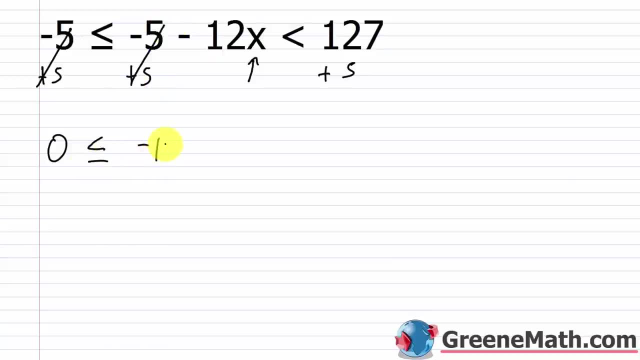 than or equal to. And then this is going to cancel. I'll just have negative 12x in the middle. And then as less than, we have 127 plus 5, that's 132. 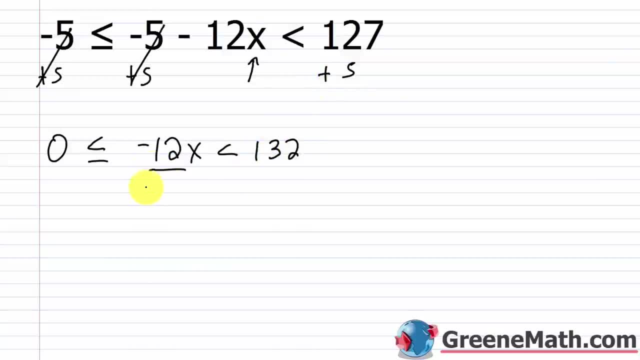 And now I'm going to divide each part by negative 12. 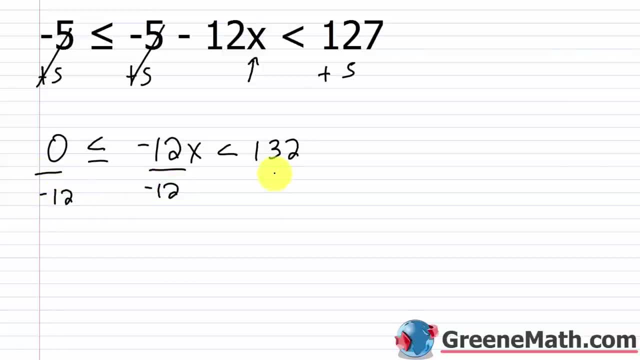 Again because I'm dividing by a negative, I've got to flip all the signs. 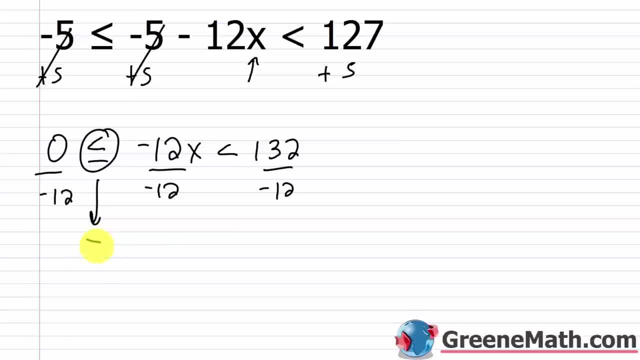 Very important. This will be a greater than or 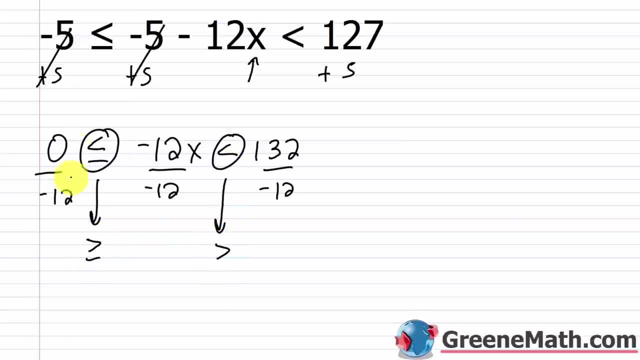 equal to. This will be a greater than. And so 0 divided by negative 12 is 0. 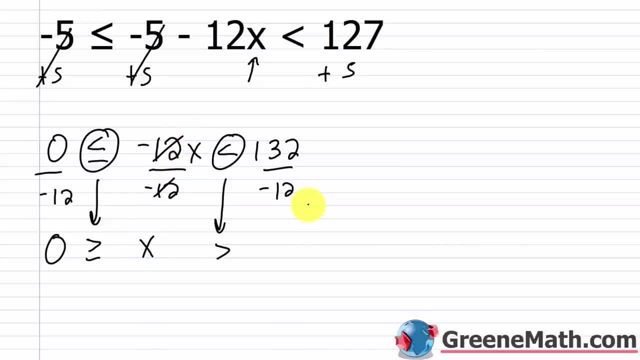 This cancels and I'll have 1 times x or just x. And then 132 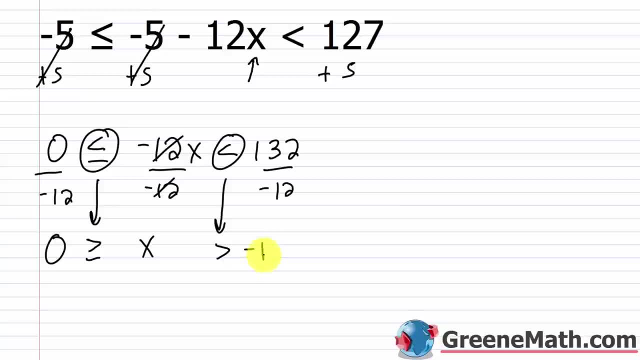 divided by negative 12 is negative 11. 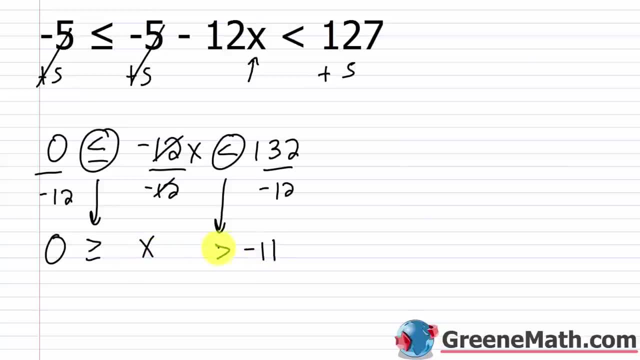 So I'm going to rewrite this in the order of the number line. So x is greater than negative 11. So I'm going to put negative 11 here. 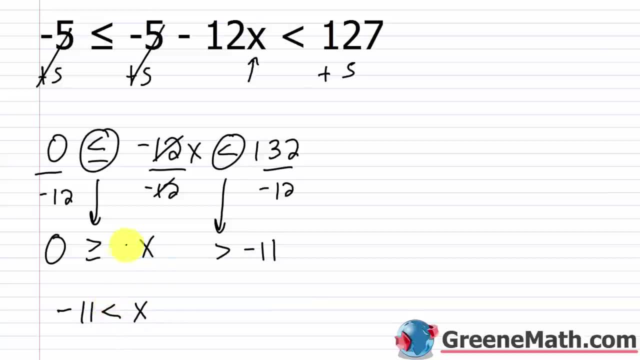 And x is greater than that. And x is less than or equal to 0. So less than or equal to 0. So x is greater than negative 11 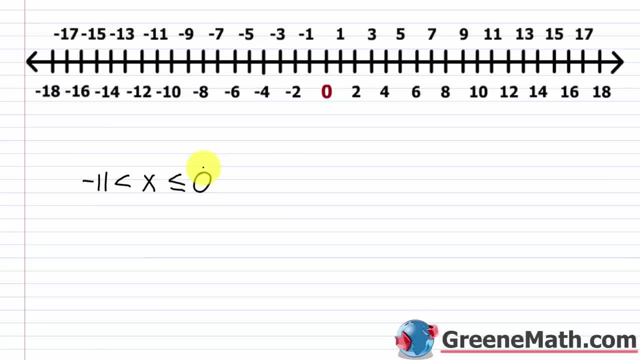 and x is less than or equal to 0. So in interval notation, my smallest value, I'm going to put negative 11. And I'm going to put a parenthesis next to it. I have a strict inequality there. x has to be strictly greater than negative 11. But up to and including 0. So my largest value is 0. And that's a non-strict inequality so I'm going to use a bracket. 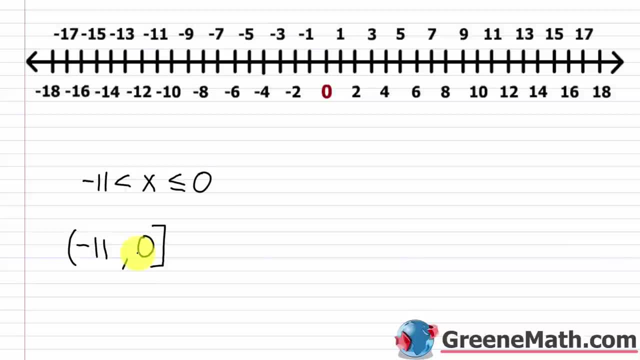 So that's my interval notation. And then graphically, I'm going to find negative 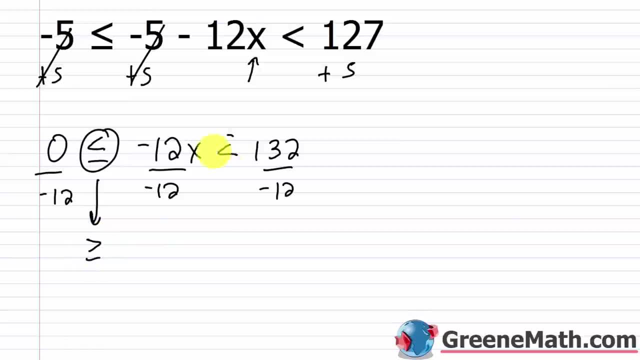 Very important. This will be a greater than or equal to. This will be a greater than, And so 0 divided by negative 12 is 0.. This cancels, and I'll have 1 times x, or just x, And then 132 divided by negative 12 is negative 11.. 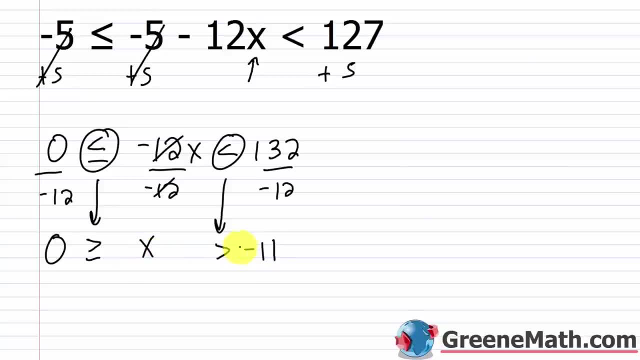 So I'm going to rewrite this in the order of the number line. So x is greater than negative 11.. So I'm going to put negative 11 here And x is greater than that, And x is less than or equal to 0.. 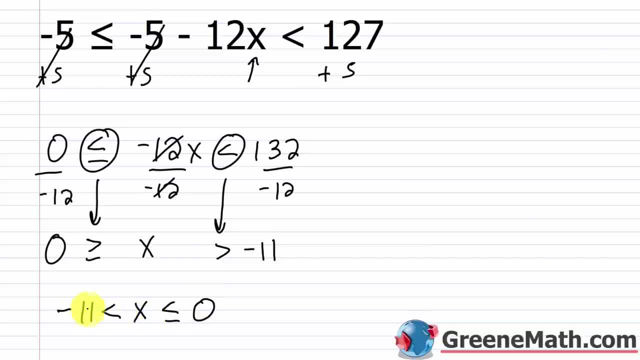 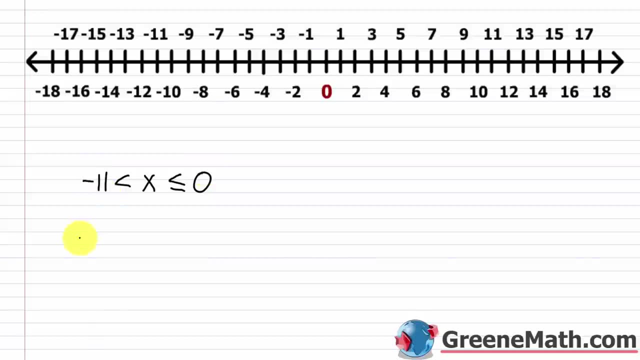 So less than or equal to 0. So x is greater than negative 11. And x is less than or equal to 0. So in interval notation, My smallest value, I'm going to put negative 11. And I'm going to put a parenthesis next to it. 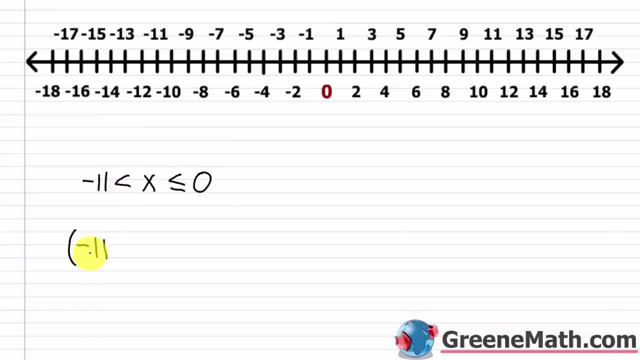 I have a strict inequality there. x has to be strictly greater than negative 11. But up to and including 0. So my largest value is 0. And that's a non-strict inequality. So I'm going to use a bracket. 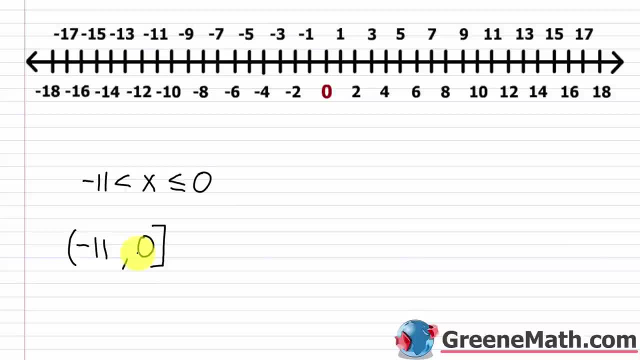 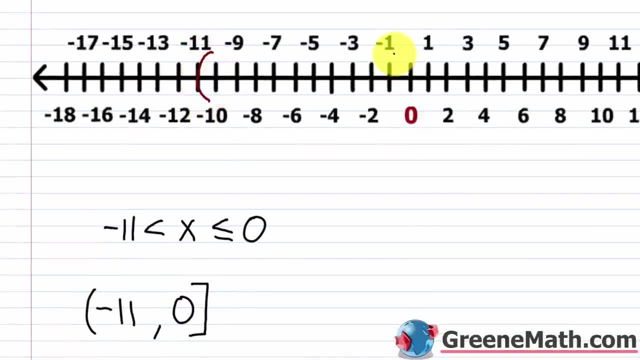 So that's my interval notation. And then graphically I'm going to find negative 11. And I'm going to put a parenthesis there. I'm going to find 0. And I'm going to put a bracket there, And then my solution- region- would be anything in between. 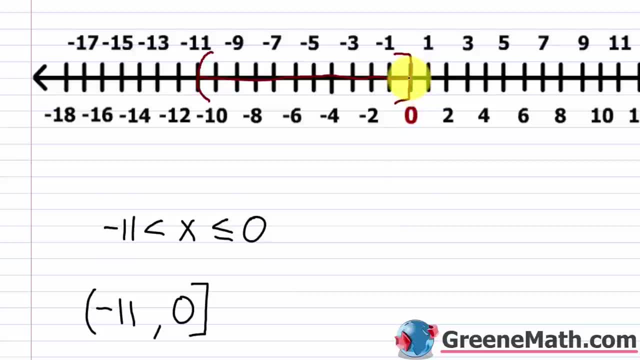 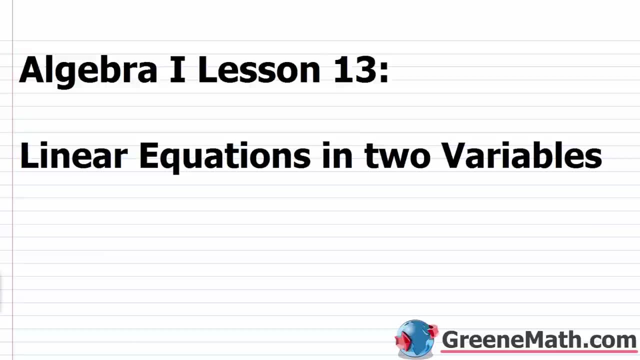 Now 0 is included, Remember, because I have a bracket, So it could be 0 or anything less Up to, but not including negative 11.. Hello and welcome to Algebra 1, Lesson 13.. In this video, we're going to learn about linear equations in two variables. 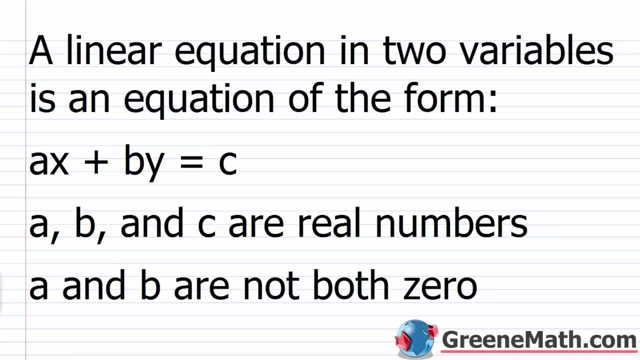 Alright. so the last chapter was all about linear equations in one variable And we also talked about linear inequalities in one variable. But now we're going to move on and talk about linear equations in two variables, In two variables. So a linear equation in two variables is an equation of the form ax plus by equals c. 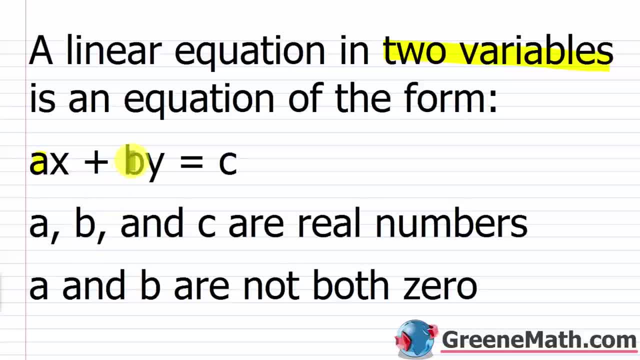 Where a, which is the coefficient of x, b, which is the coefficient of y, And c, which is a constant term, are real numbers. And again, I know I haven't given you an official definition, for you know what a real number is, But it's, at this point, any number you can think of. 11. And I'm going to put a parenthesis there. I'm going to find 0. And I'm going to put a bracket there. 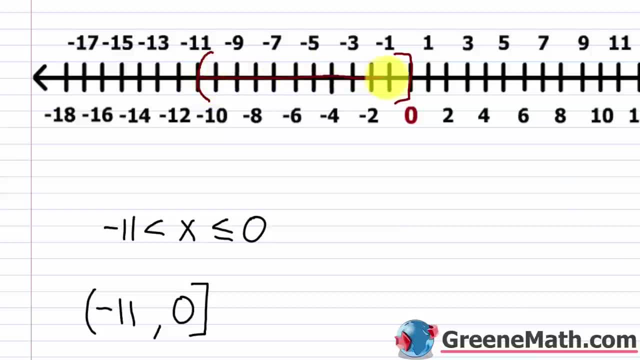 And then my solution region would be anything in between. 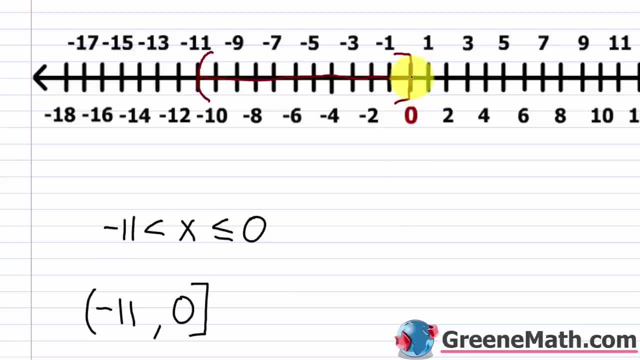 Now 0 is included. Remember because I have a bracket. So it could be 0 or anything less up to but not including negative 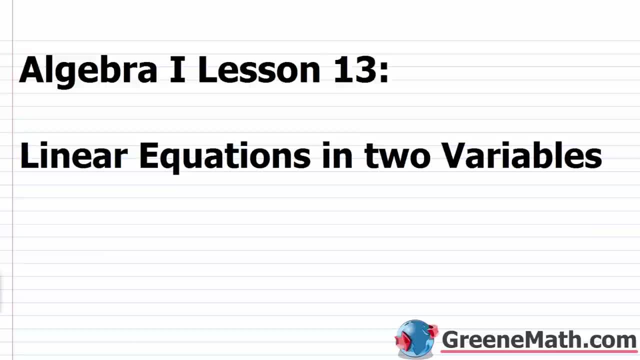 Hello and welcome to Algebra 1 Lesson 13. In this video we're going to learn about linear equations in two variables. 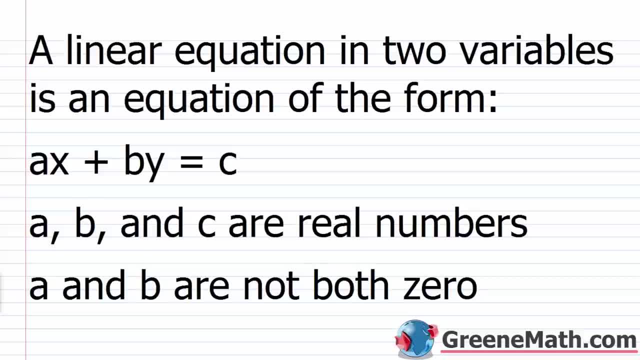 Alright so the last chapter was all about linear equations in one variable and we also talked about linear inequalities in one variable but now we're going to move on and talk about linear equations 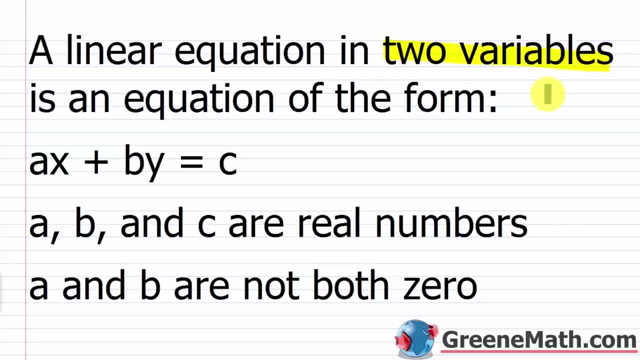 In two variables. So a linear equation in two variables is an equation of the form ax plus by equals c. Where a which is the coefficient of x b which is the coefficient of y and c which is a constant term are real numbers. 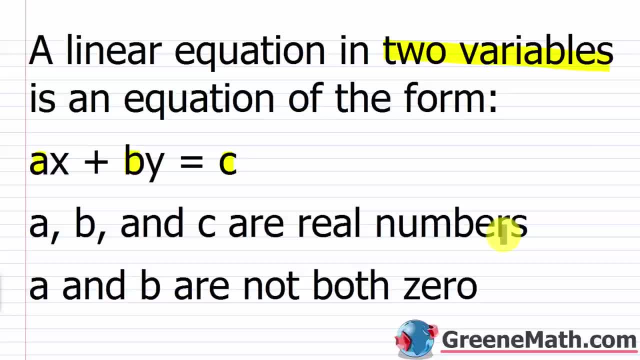 And again I know I haven't given you an official definition for what a real number is but it's at this point any number you can think of. So I could put fractions there, decimals, negatives, doesn't really matter. Anything you can think of at this point could go in there. But there is a restriction. 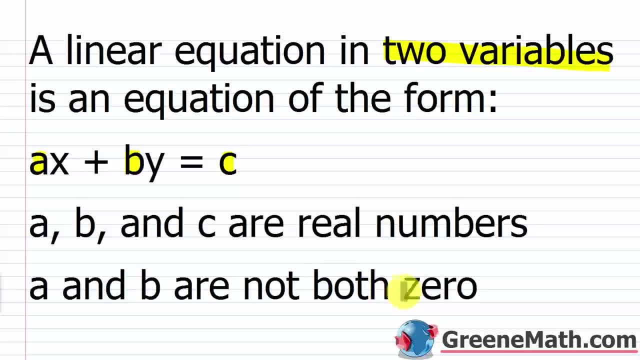 We say that a and b are not both 0. So these are the coefficients for our variables. 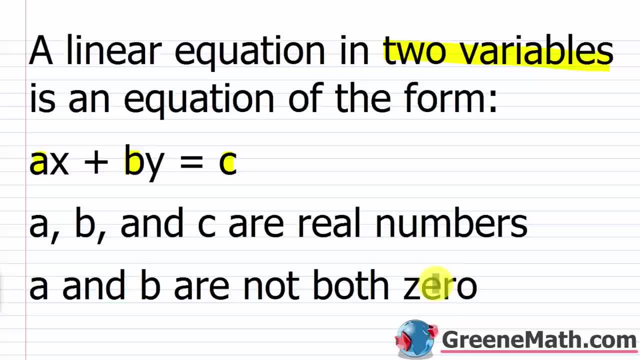 So we can't have both of them 0 at the same time. I could have one of them be 0 but the other one could not be 0. So here are some examples. 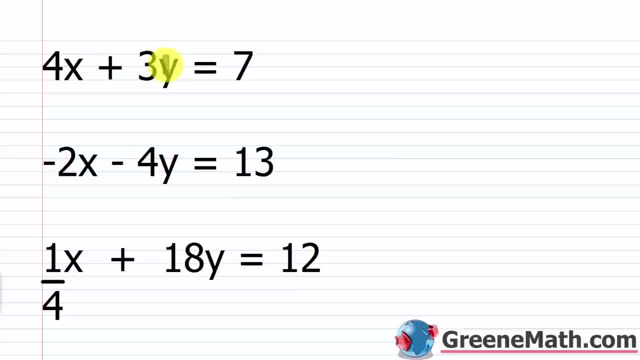 We have 4x plus 3y equals 7. So you see you have two variables here. You have an x variable and a y variable. We have negative 2x minus 4y equals 13. Again two variables here. You have an x variable and a y variable. And then 1 fourth x plus 18y equals 12. Again x and 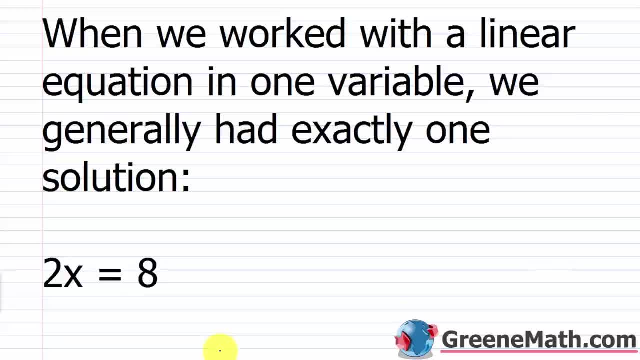 then y. So when we work with a linear equation and one variable we generally had exactly one 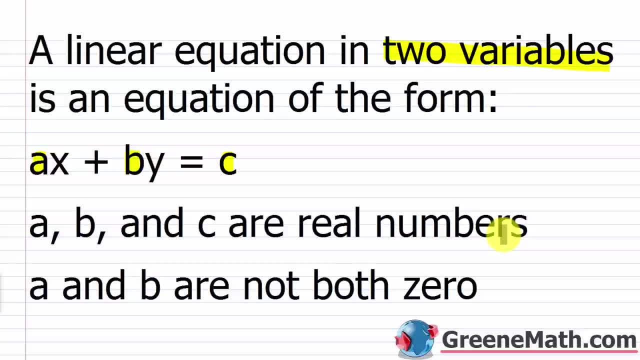 So I could put fractions there, decimals, you know, negatives Doesn't really matter. Anything you could think of at this point could go in there, But there is a restriction. We say that a and b are not both 0.. So these are the coefficients for our variables. 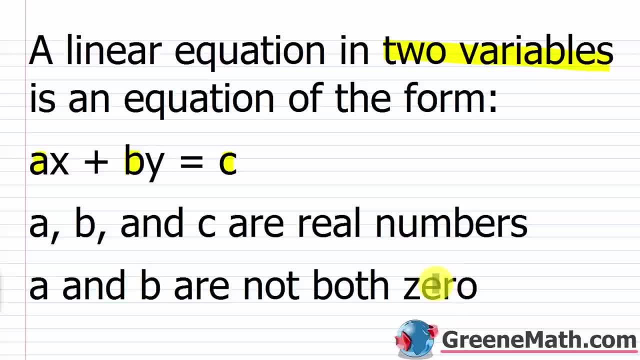 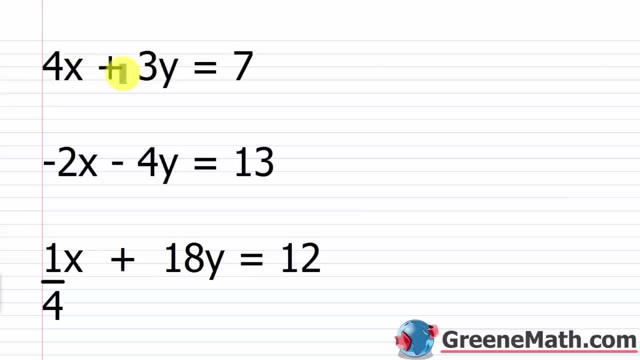 So we can't have both of them 0 at the same time. I could have one of them be 0, but the other one could not be 0. So here are some examples. We have: 4x plus 3y equals 7.. 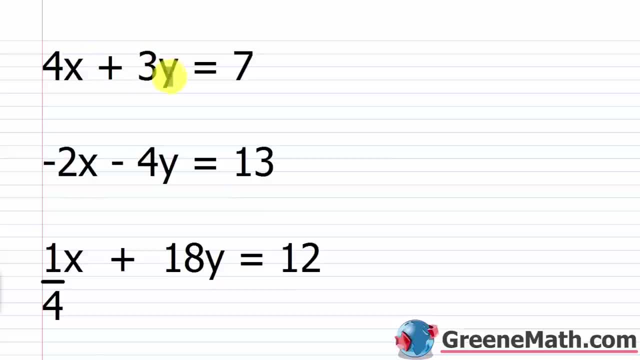 So you see, you have two variables here. You have an x variable and a y variable. We have negative. 2x minus 4y equals 13.. Again two variables here. You have an x variable and a y variable. And then 1 fourth x plus 18y equals 12.. 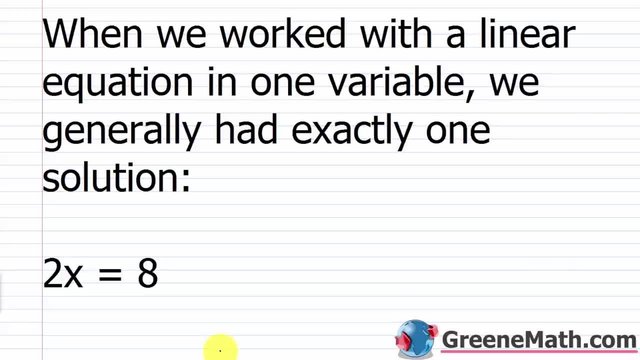 Again x and then y. So when we worked with a linear equation in one variable, we generally had exactly one solution- And I know we talked about a special case scenario where that's not going to be true, But in general we had one solution. 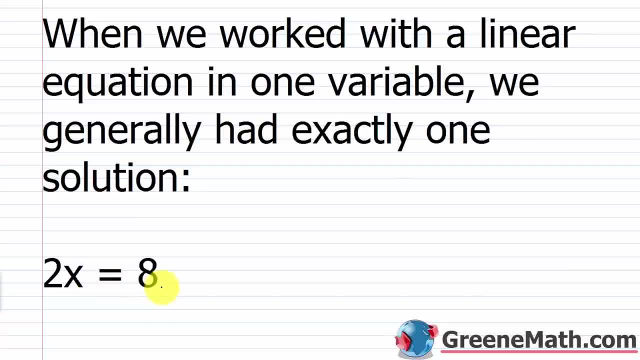 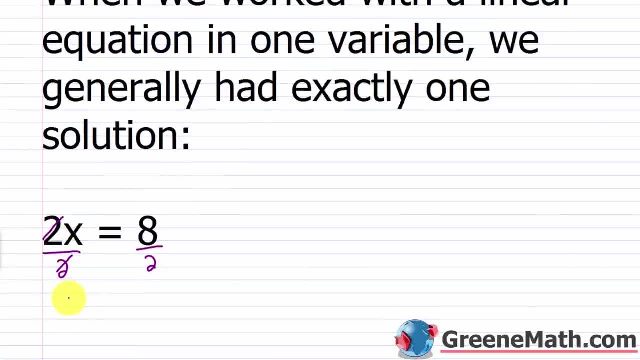 So if I looked at something like, 2x equals 8.. We already know how to solve this. We divide both sides of the equation by 2.. Which is the coefficient of x. This cancels with this And I just have: x equals a. divided by 2 is 4.. 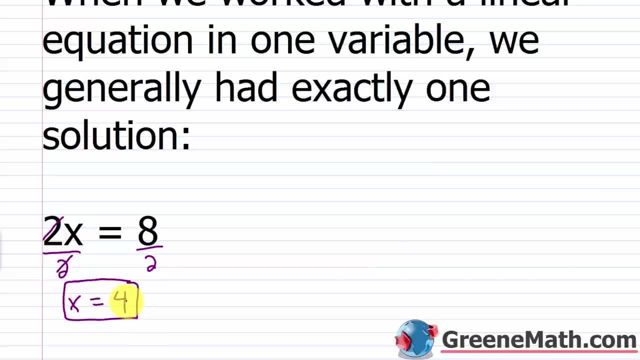 So there's exactly one solution here: There's only one number that, when plugged in for x, gives us a true statement. And what we're going to see when we start working with linear equations in two variables is that there's an infinite number of x- y combinations that are going to make the equation. 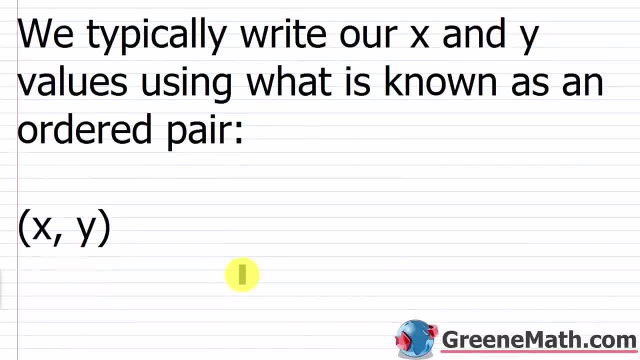 true. So let's talk a little bit about how to write a solution for a linear equation in two variables. So we typically write our x and y values using what is known as an ordered pair. So you might want to write that down because it's an extremely important vocabulary term. 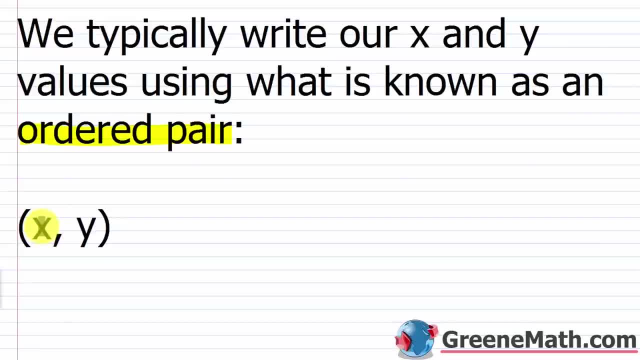 An ordered pair Looks like this: You have an x comma, a, y, So all the way on the left is always your x value, Your x value, And then on the right is always your y value. These are not interchanged Ever. solution. And I know we talked about a special case scenario where that's not going to 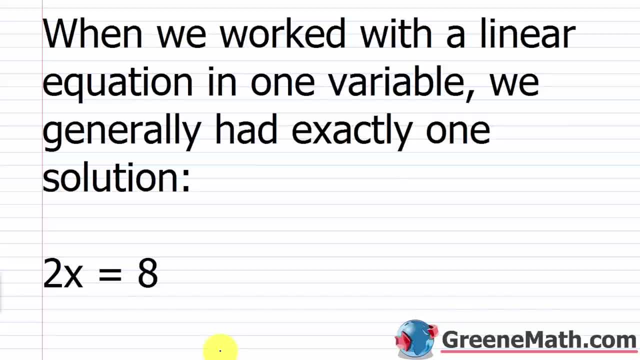 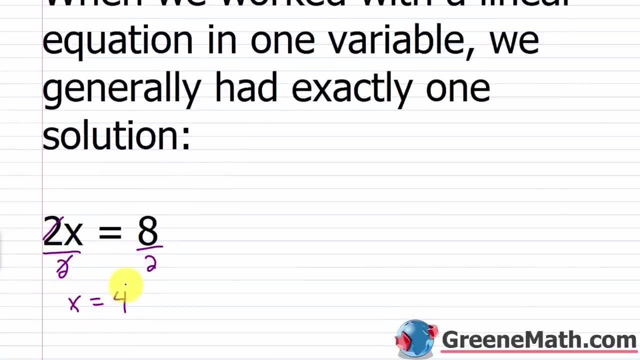 be true. But in general we had one solution. So if I looked at something like 2x equals 8 we already know how to solve this. We divide both sides of the equation by 2 which is the coefficient of x. This cancels with this. And I just have x equals 8 divided by 2 is 4. 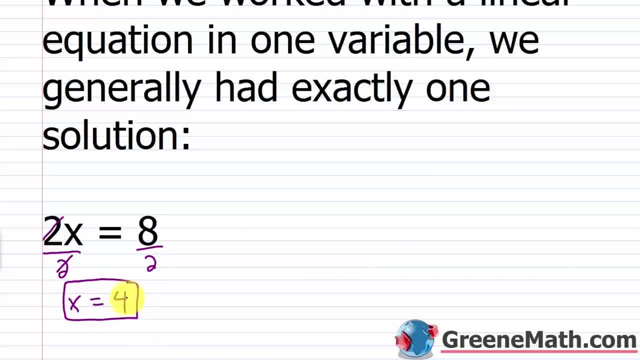 So there is exactly one solution here. There is only one number. That when plugged in for x gives us a true statement. 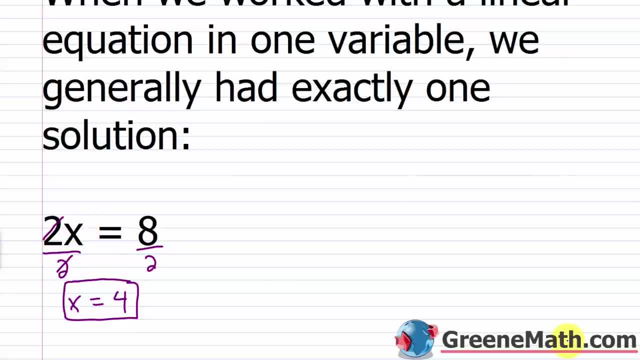 And what we are going to see when we start working with linear equations and two variables is that there is an infinite number of x y combinations that are going to make the equation true. So let's talk a little bit 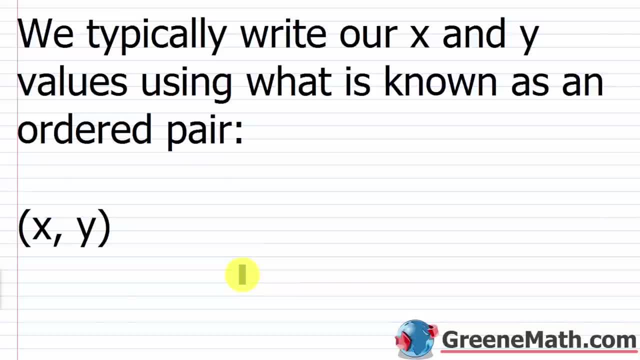 about how to write a solution for a linear equation and two variables. 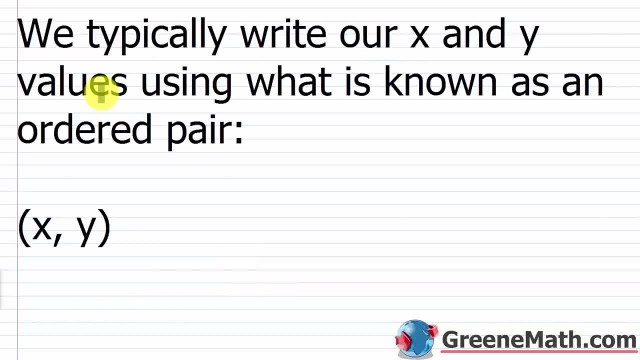 So we typically write our x and y values using what is known as an ordered pair. So you might want to write that down because it's an extremely important vocabulary term. An ordered pair looks like this. You have an x comma a y. 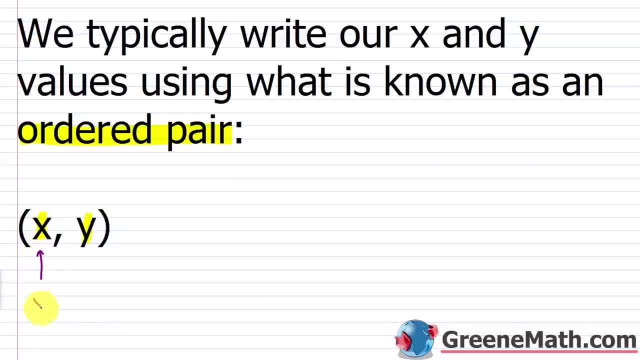 So all the way on the left is always your x value. Your x value. 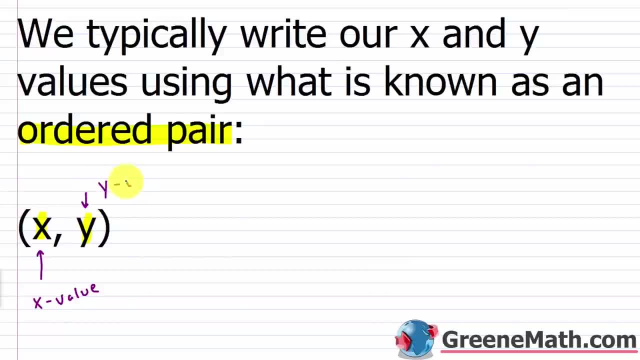 And then on the right is always your y value. 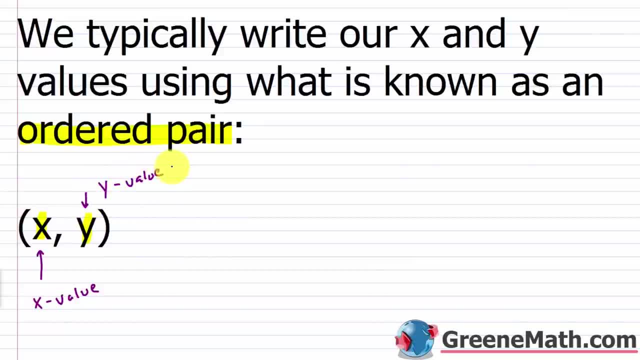 These are not interchanged. Ever. It's always the x value comma the y value. 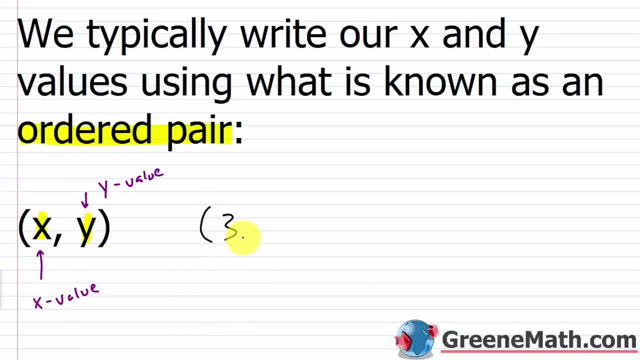 So in other words if I give you an ordered pair 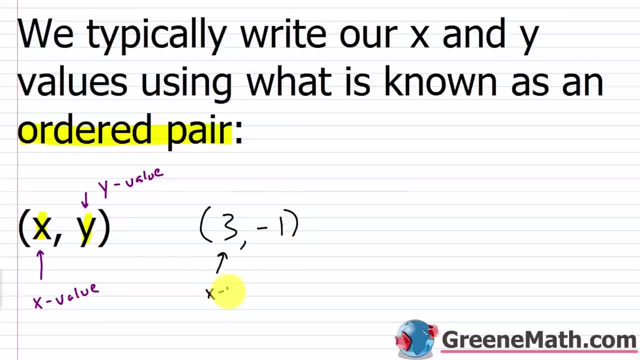 3 comma negative 1 is your x value. 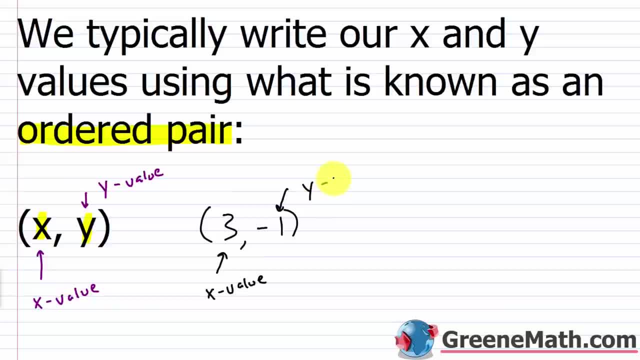 And negative 1 is your y value. 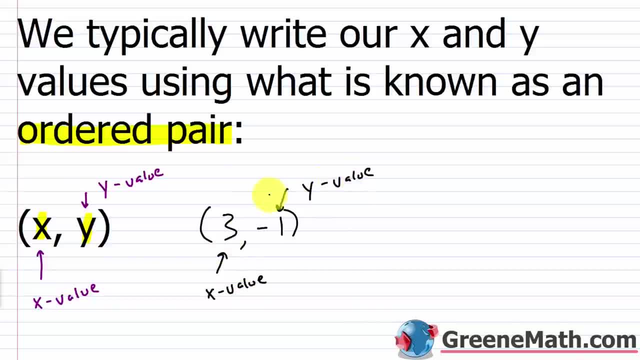 So again the x value is on the left. The y value is on the right. 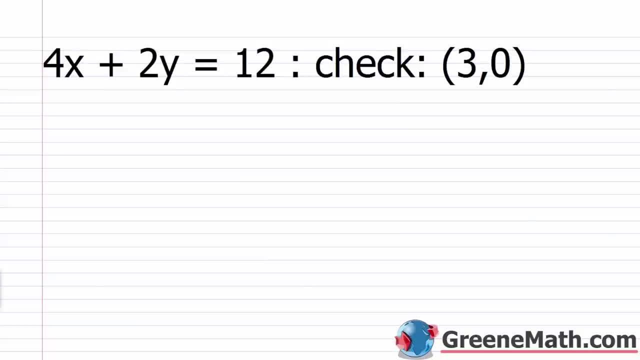 Alright so now let me show you how to check an ordered pair and see if it's a solution to a linear equation and two variables. 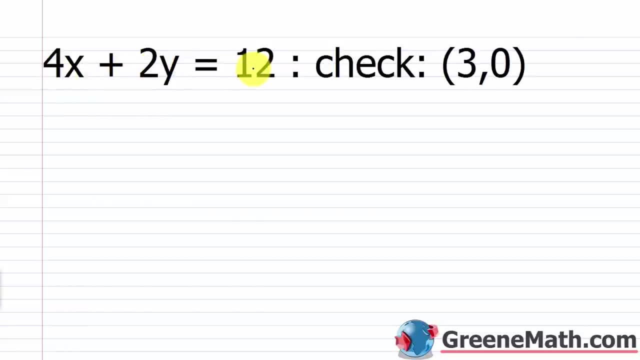 So we have this 4x plus 2y equals 12. And we want to check the ordered pair 3 comma 0. 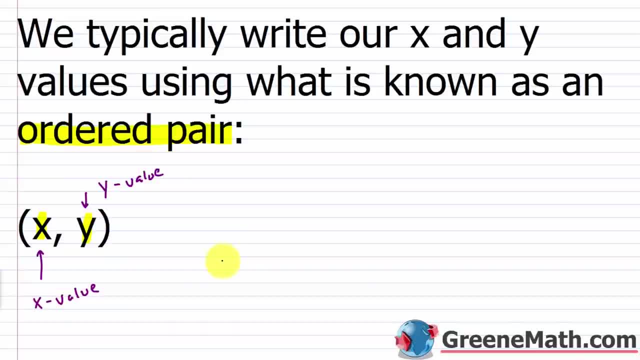 It's always the x value comma the y value. So in other words, if I give you an ordered pair, 3, comma negative 1.. 3 is your x value And negative 1 is your y value. So again, the x value is on the left. 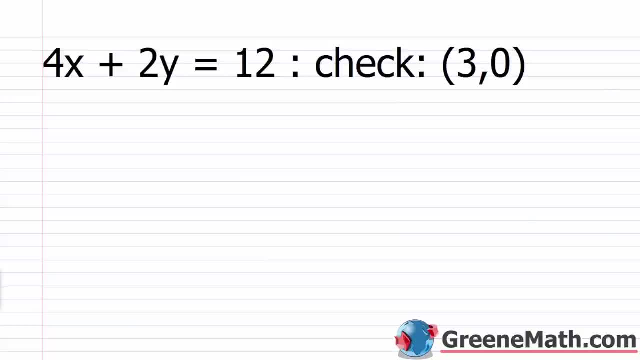 The y value is on the right. Alright, so now let me show you how to check an ordered pair and see if it's a solution to a linear equation in two variables. So we have this: 4x plus 2y equals 12.. 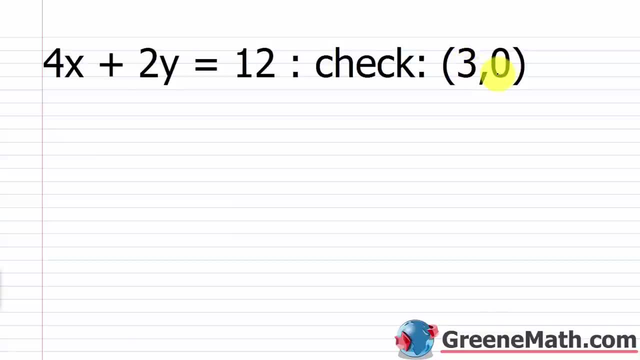 And we want to check the ordered pair 3 comma 0.. So the important thing to remember is that, again, the left value Is the x value And the right value is the y value. Very, very important. you understand that. So, just like we did with a linear equation of one variable, 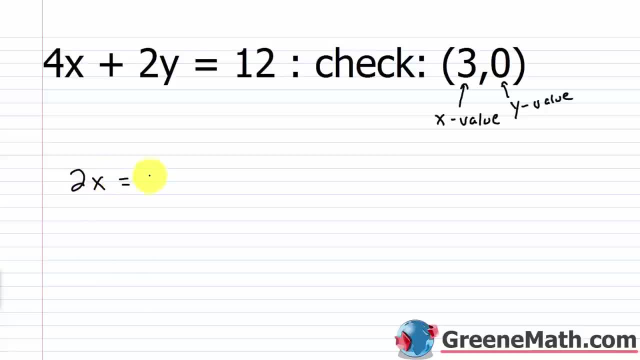 So, for example, if I have 2x equals 8.. Like we had earlier And I said, x is equal to 4.. Alright, this was the solution. I plug a 4 in for x. So 2 times 4 equals 8.. 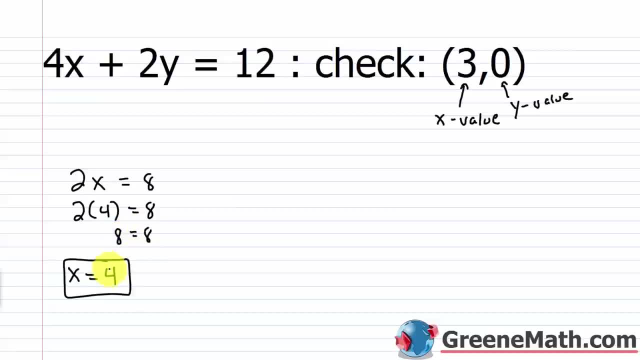 And we see that the left and the right side are equal 8.. 8 equals 8.. That's how I know that x equals 4 is the solution. Well, it's the same here. All I'm going to do is take each number. 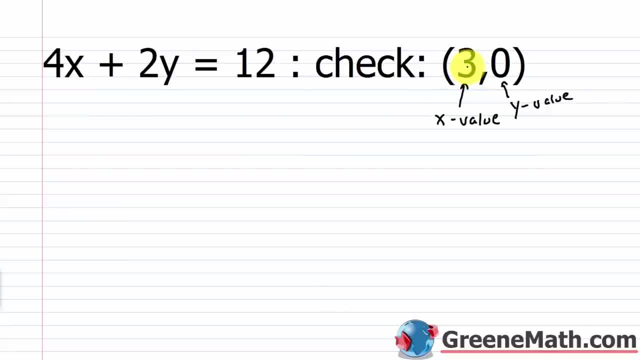 And plug it in for its respective variable. So 3 will get plugged in for x Because it represents the x value. 0 will get plugged in for y Because it represents the y value. So I would have 4 times. Again, I have an x here. 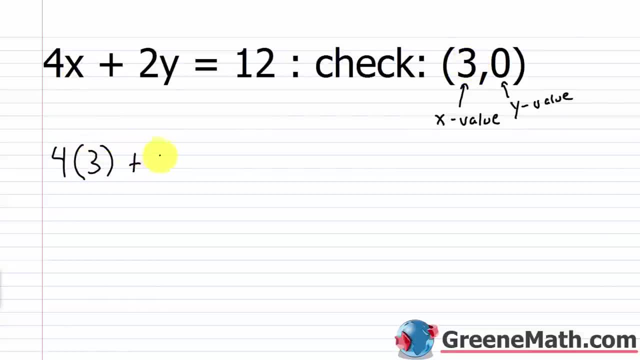 This is my x value, So I'm going to put a 3.. Plus 2 times 0 is my y value. I'm putting in a 0 for y equals 12.. Very, very simple. I'm just plugging in, just like I did with a linear equation in one variable. 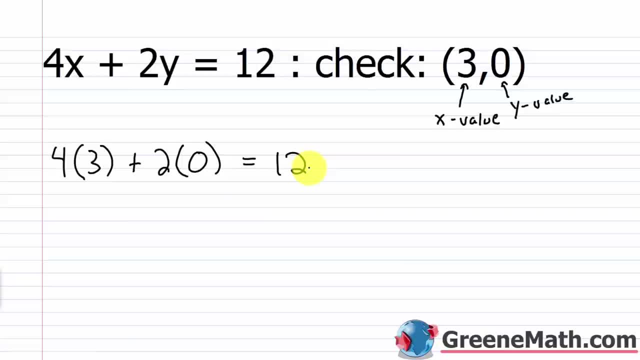 If I have the solution there. I plugged in for x. I found out if the left and the right side were equal. I'm doing the same thing here. I'm just including another variable. I now have two of them, So 4 times 3 is 12.. 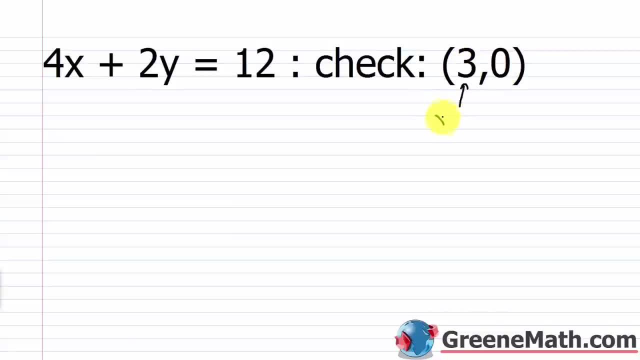 So the important thing to remember is that again the left value is the x value. 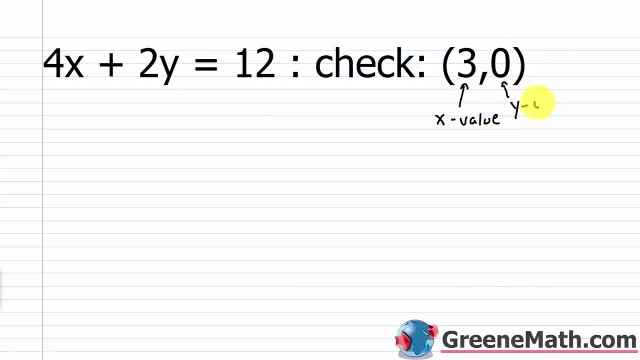 And the right value is the y value. Very very important you understand that. 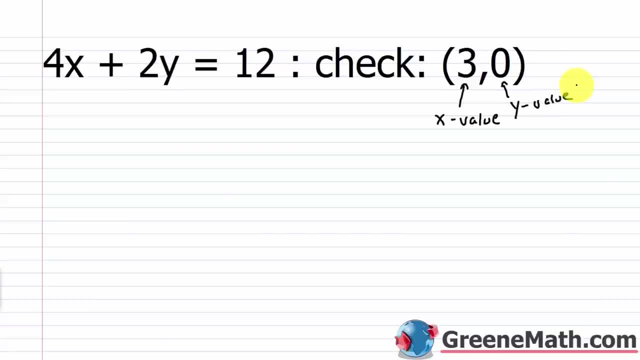 So just like we did with a linear equation of one variable. So for example if I have 2x equals 8. Like we had earlier. And I said x is equal to 4. Alright this was the solution. I plug a 4 in for x. So 2 times 4 equals 8. 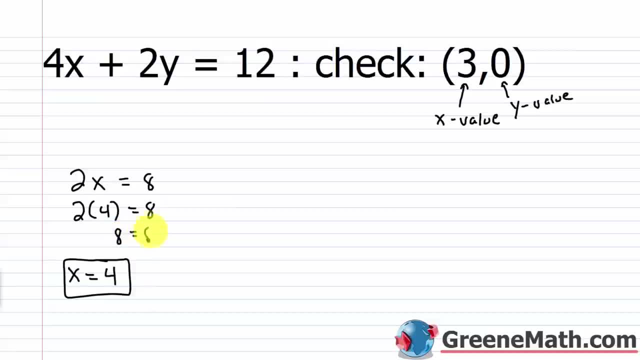 And we see that the left and the right sides are equal. 8 equals 8. That's how I know that x equals 4 is the solution. 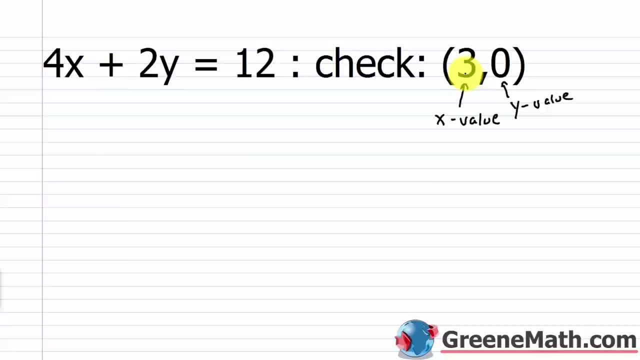 Well it's the same here. All I'm going to do is take each number and plug it in for its respective variable. So 3 will get plugged in for x because it represents the x value. 0 will get plugged in for y because it represents the y value. So I would have 4 times again I have an x here. This is my x value. So I'm going to put a 3. 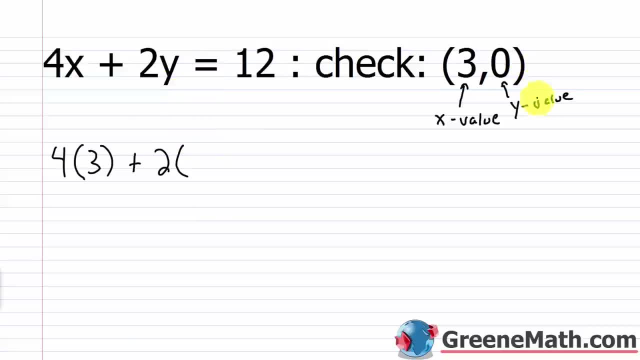 Plus 2 times. 0 is my y value. So I'm putting in a 0 for y. Equals 12. 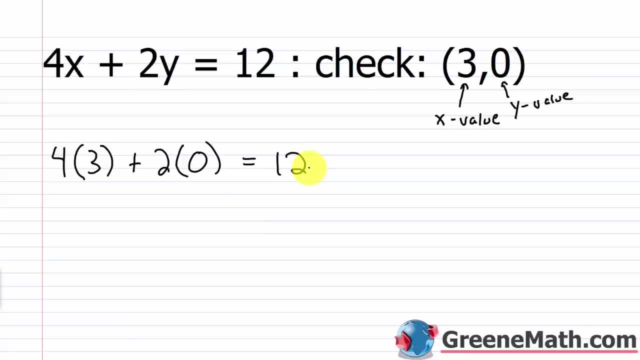 Very very simple. I'm just plugging in just like I did with a linear equation of one variable. 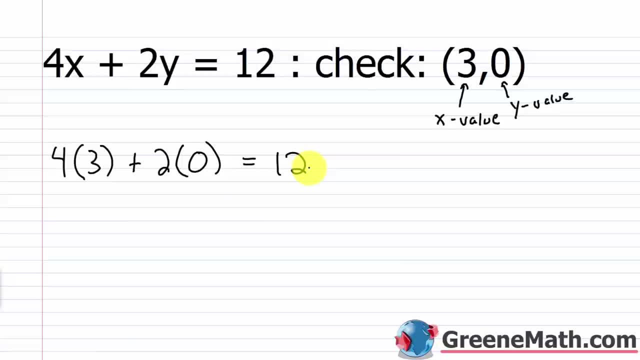 If I had the solution there I plugged in for x. I found out if the left and the right side were equal. I'm doing the same thing here. I'm just including another variable. I now have two of them. So 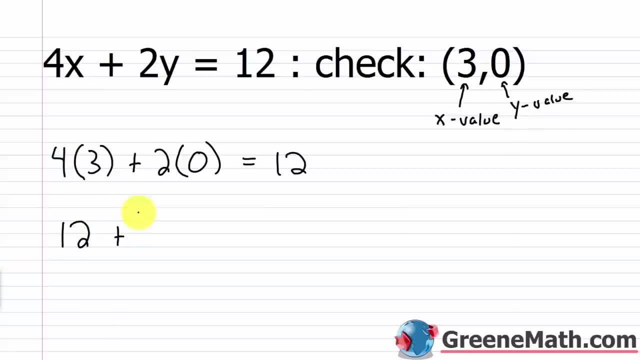 4 times 3 is 12. Plus 2 times 0 is 0. So I can put plus 0 or I could just leave it as 12. And this is supposed to equal 12. And it does. We get the same value on the left and the right side. And so we can say this ordered pair 3 comma 0 is a solution for our equation. 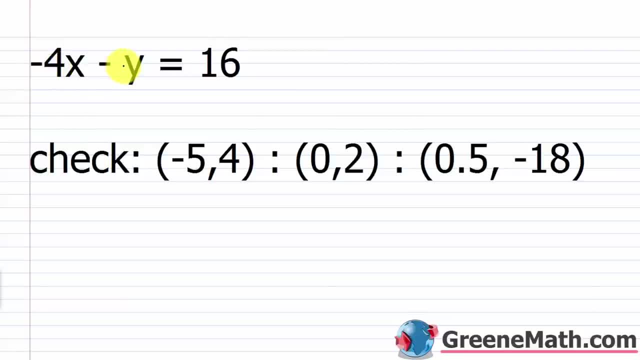 Alright let's take a look at some problems now. We have negative 4x minus y equals 16. And we're going to check each ordered pair and see if it's a solution to the equation. So we have our first ordered pair which is negative 5 comma 4. Again the left value is the x value. The x value. The right value is 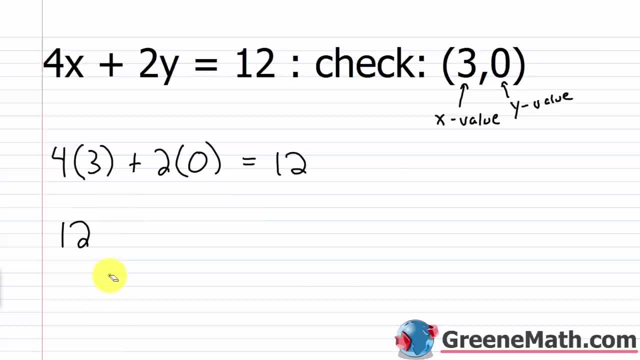 Plus 2 times 0 is 0. So I can put plus 0 or I could just leave it as 12. And this is supposed to equal 12. And it does. We get the same value on the left and the right side. 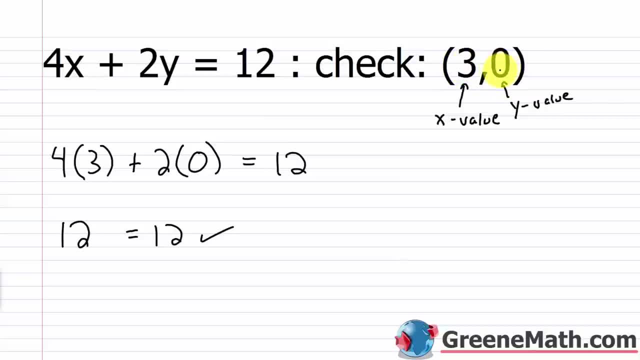 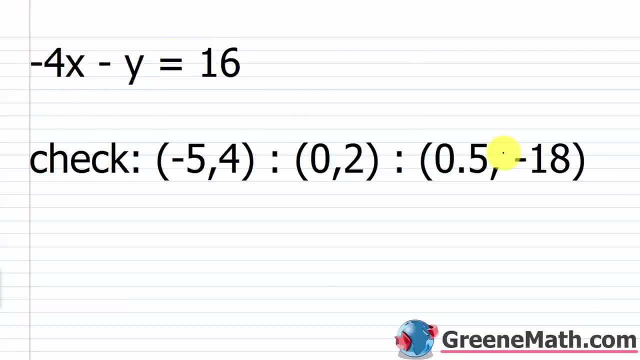 And so we can say this ordered pair 3 comma 0 is a solution for our equation. Alright, let's take a look at some problems. now We have negative. 4x minus y equals 16. And we're going to check each ordered pair. 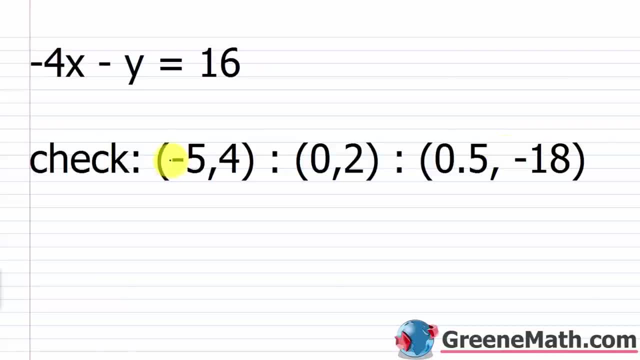 And see if it's a solution to the equation. So we have our first ordered pair which is negative, 5 comma 4.. Again, the left value is the x value, The x value, The right value is the y value, So we have negative 4x. 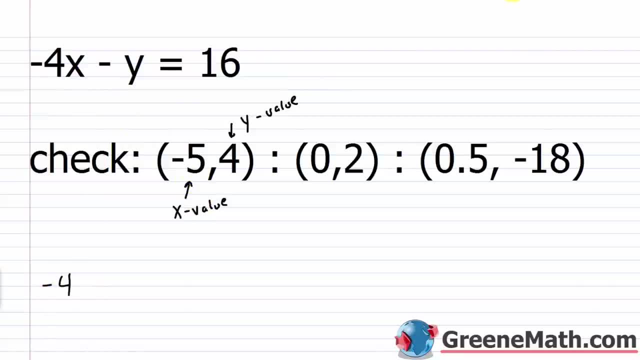 So instead of x, I'm going to plug in a negative 5.. This is what I'm plugging in for x. So negative 4 times negative, 5 minus. Now I have a y And I'm plugging in a 4 for y. 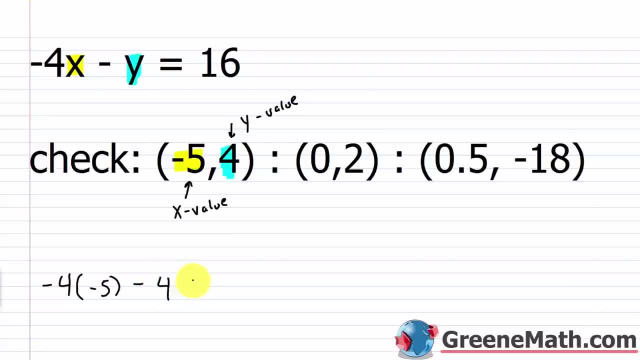 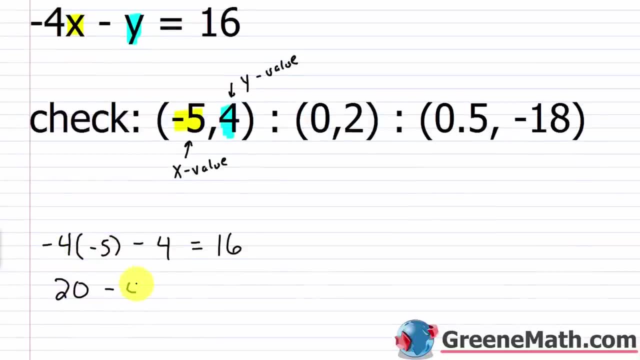 Because that's my y value. So minus 4.. And this equals 16.. So negative 4 times negative, 5 is 20.. And minus 4 equals 16.. 20 minus 4 is 16. So you get 16 equals 16.. 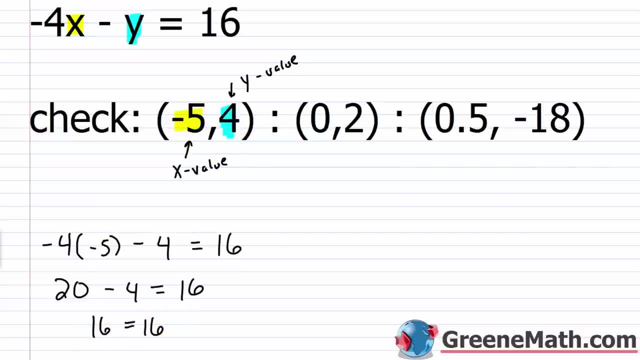 So, yes, this ordered pair, negative 5 comma 4, is a solution, So I'm just going to put a check mark here, Alright, the next ordered pair we're going to look at is 0 comma 2.. And again, we have our left value as our x value. 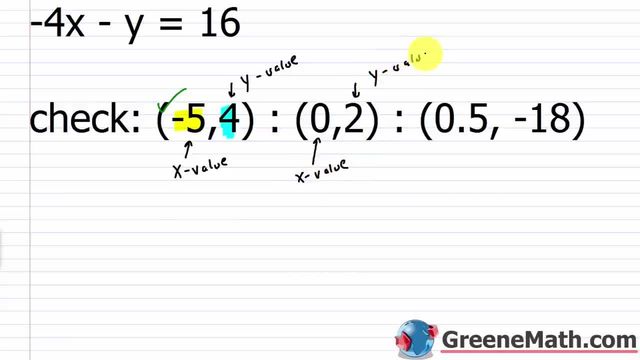 Our right value is the y value And that's not going to change. Okay, you just memorize that. The one on the left is the x, The one on the right is the y, The one on the right is the y, So we have negative 4 times. our x value is 0.. 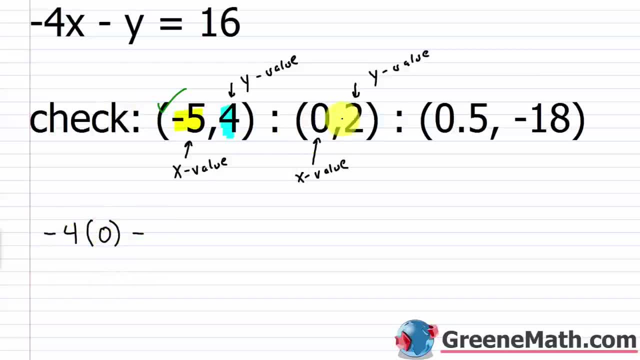 So I'm going to plug in a 0 there. Minus our y value is 2 equals 16.. Negative 4 times 0 is 0. So then minus 2 equals 16.. So we get negative 2 equals 16.. 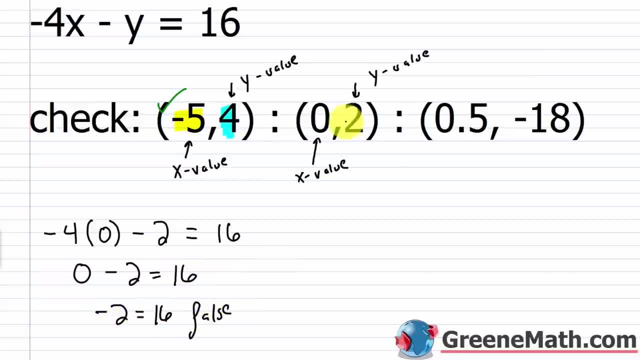 And that's not true. This is false. So this does not work as a solution. So this doesn't work. Alright, let's try the ordered pair: 0.5 comma negative 18.. So again, the left value is the x value. 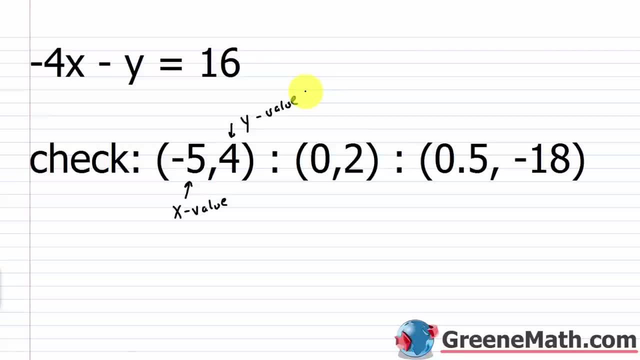 the y value. So we have negative 4x. So instead of x I'm going to plug in a negative 5. This is what I'm plugging in for x. So negative 4 times negative 5 minus now I have a y. 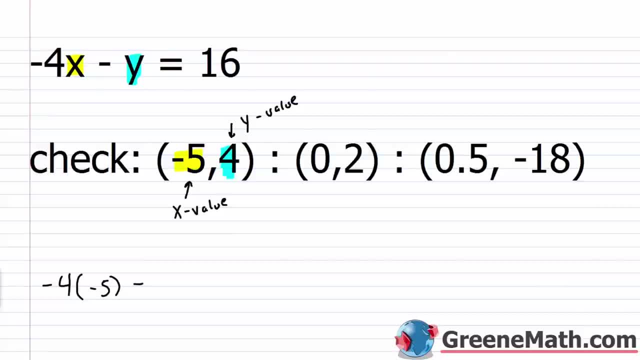 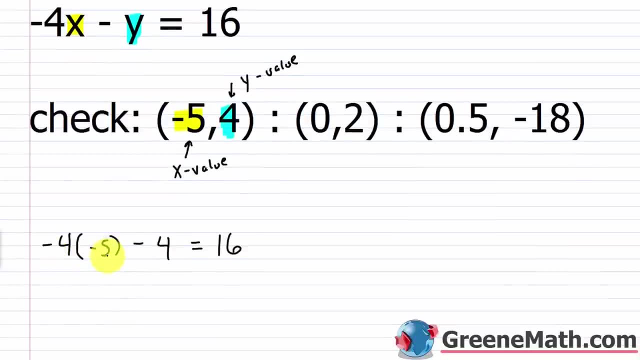 And I'm plugging in a 4 for y. Because that's my y value. So minus 4 and this equals 16. So negative 4 times negative 5 is 20. And minus 4 equals 16. 20 minus 4 is 16. So you get 16 equals 16. So yes this ordered 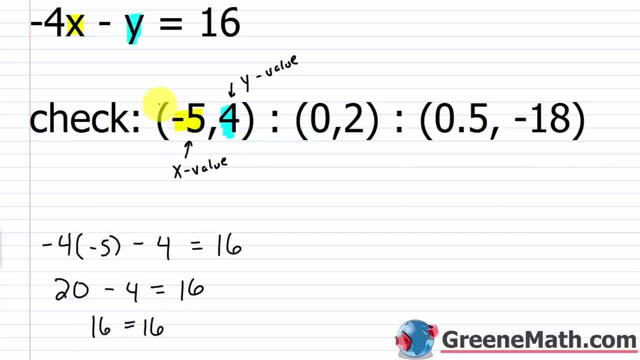 pair negative 5 comma 4 is a solution. So I'm just going to put a check mark here. Alright the next ordered pair we're going to look at is 0 comma 2. 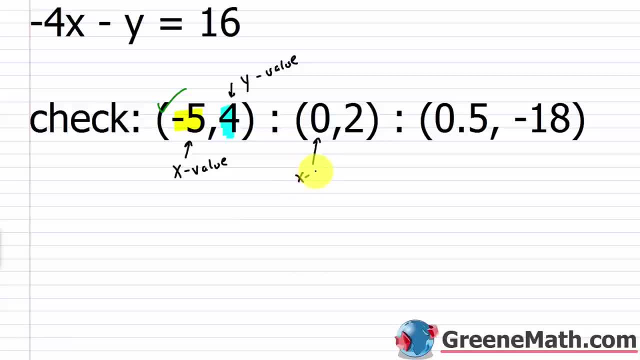 And again we have our left value as our x value. 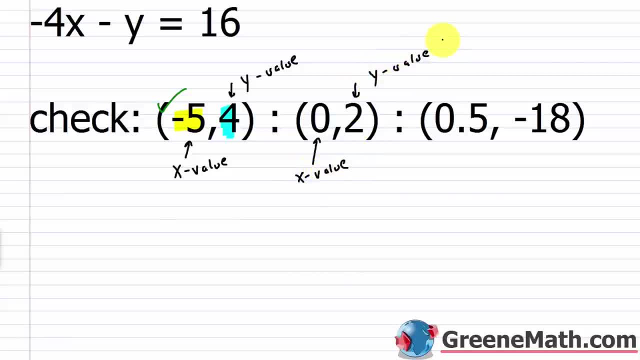 Our right value is the y value. And that's not going to change. 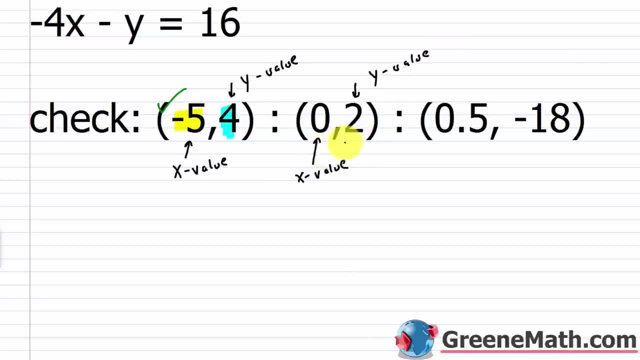 You just memorize that. The one on the left is the x. The one on the right is the y. 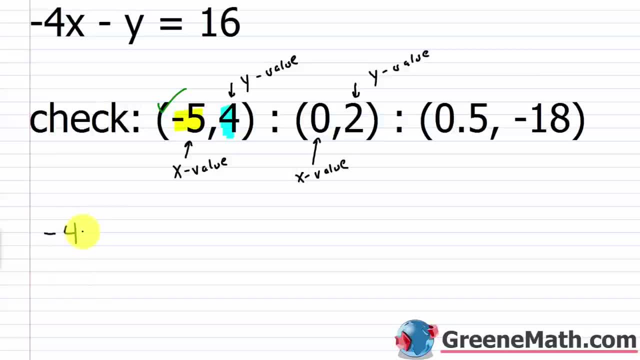 So we have negative 4 times our x value is 0. So I'm going to plug in a 0 there. 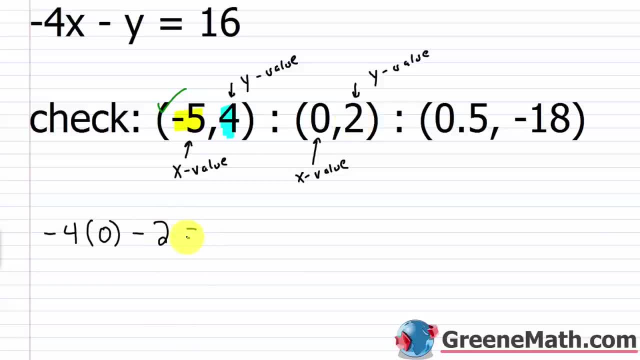 Minus our y value is 2 equals 16. Negative 4 times 0 is 0. So then minus 2 equals 16. So we get negative 2 equals 16. And that's not 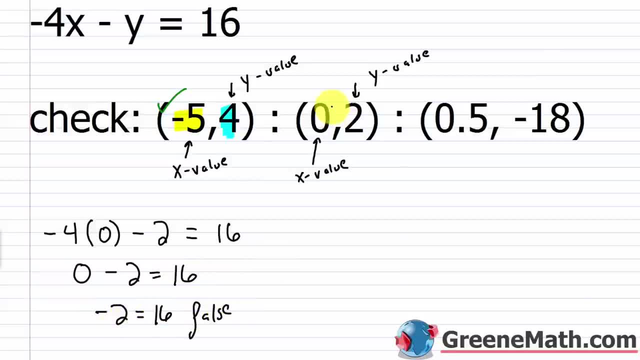 true. This is false. So this does not work as a solution. So this doesn't work. 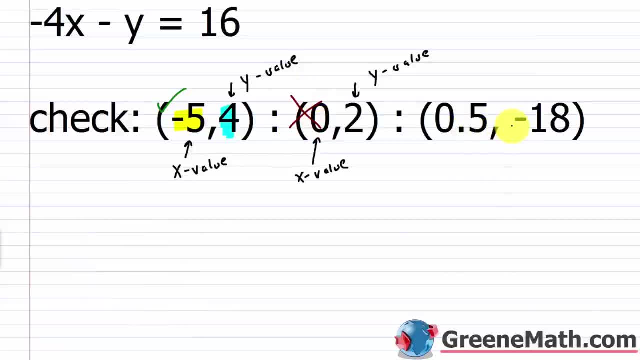 Alright let's try the ordered pair 0.5 comma negative 18. 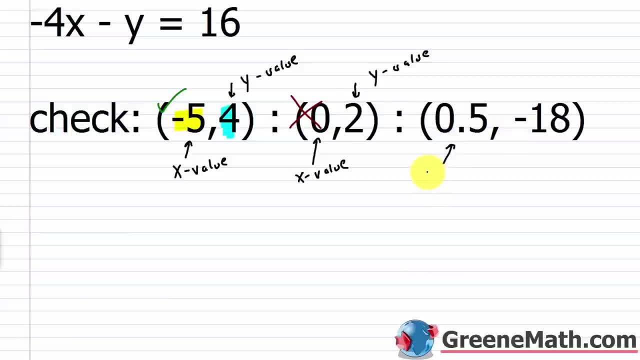 So again. The left value is the x value. The x value. And the right value is the y value. 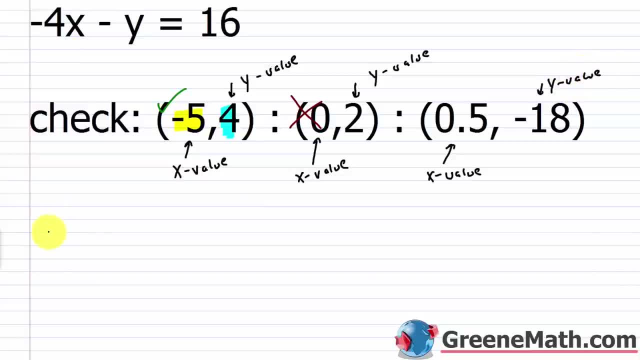 So we're just going to plug in. We'll have negative 4 times x. And again x is going to be 0.5. Or that's 1 half. Whatever you want to put in there. Minus. For y 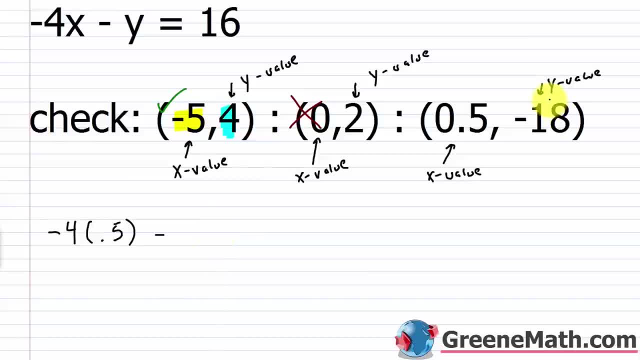 we have negative 18. And this is very important. When you're plugging in for something this is negative 18 that I'm plugging in here for y. 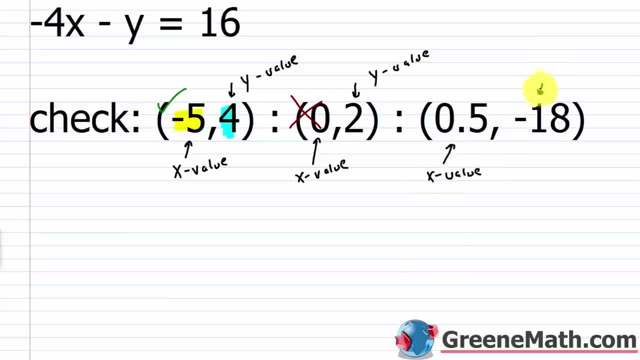 The x value And the right value is the y value. So we're just going to plug in: We'll have negative 4 times x And again x is going to be 0.5. Or that's 1 half, or whatever you want to put in there. 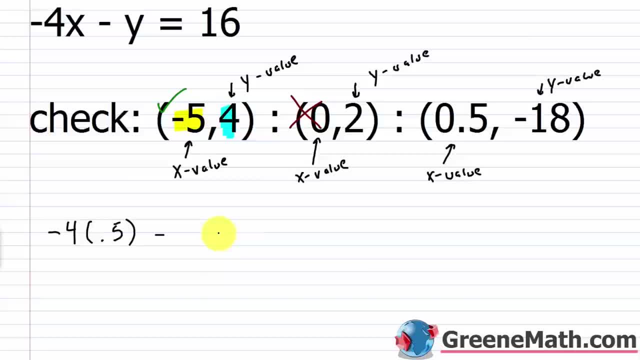 Minus For y, we have negative 18.. And this is very important When you're plugging in for something. This is negative 18 that I'm plugging in here for y. This is negative 18 that I'm plugging in here for y. 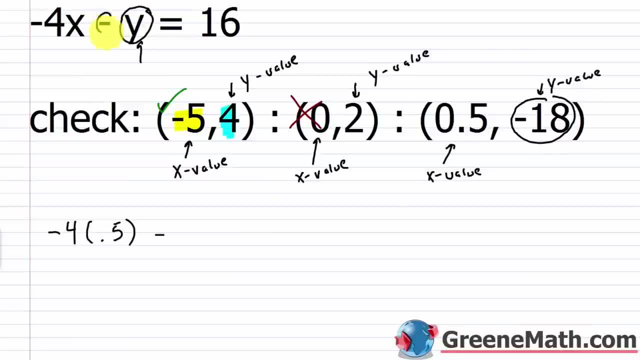 there's a minus sign already out in front, so this stays there, and then you put minus 18 or negative 18, and minus a negative is plus a positive, so i can write minus a negative 18, or i could simplify that and put plus positive 18, which i'm going to do in the next step. so equals 16, so what's negative? 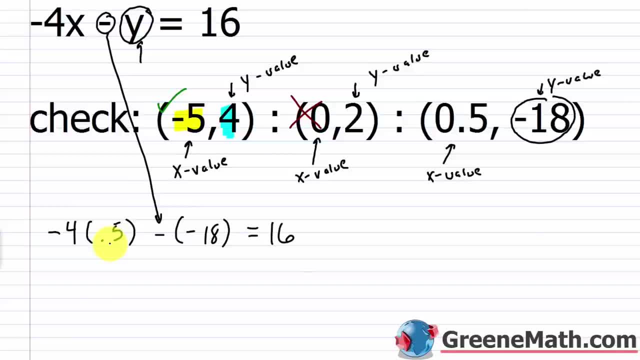 4 times 0.5 again. you could do that using negative 4 times 1 half and kind of mentally say: okay, well, negative 4 times 1 half is negative 2. so this is negative 2 minus the negative 18 is plus 18. 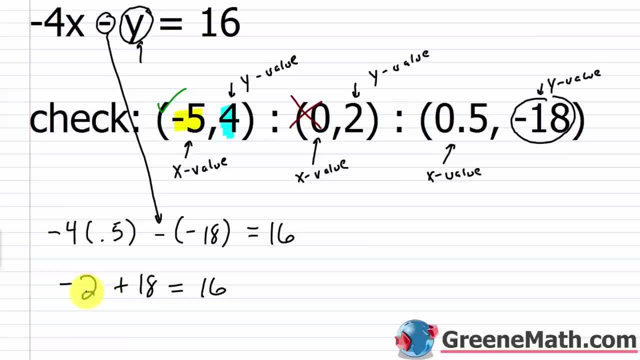 equals 16, and so, yeah, this is going to be true. negative 2 plus 18 is 16. 16 does equal 16. same value on each side of the equation, and so we're going to check, mark this and say, yes, it is a solution to the equation. and one thing this would immediately draw your attention to is the fact. 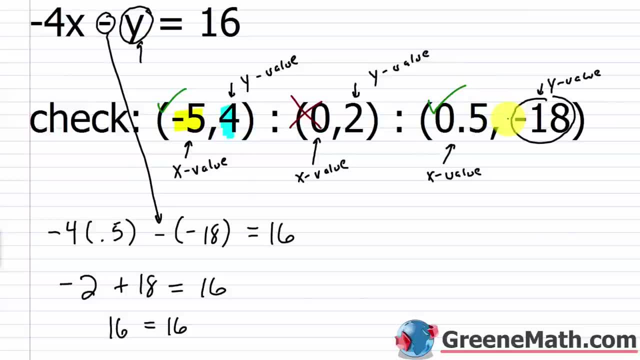 that again, we can have more than one. you can have more than one ordered pair. that works as a solution to a linear equation in two variables when we worked with a linear equation in one variable. generally speaking, we're going to have exactly one value for our variable. that makes the equation true. here we have multiple ordered pairs or multiple solutions here. 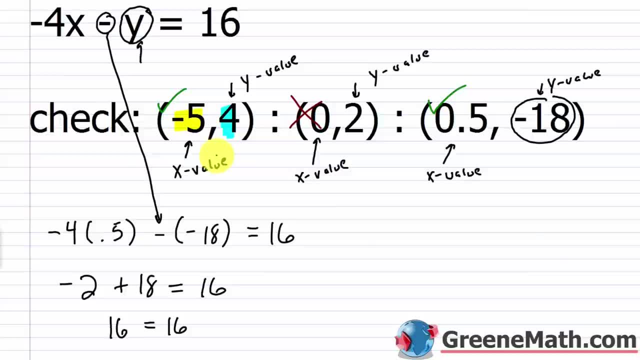 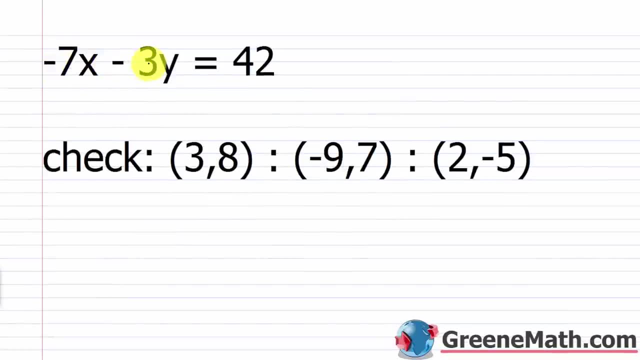 that work and in fact you're going to find that with a linear equation in two variables there's an infinite number of ordered pair solutions. all right, so now we're going to look at negative: 7x minus 3y equals 42 and we want to check the ordered pair 3 comma 8, the ordered pair negative 9 comma 7, and. 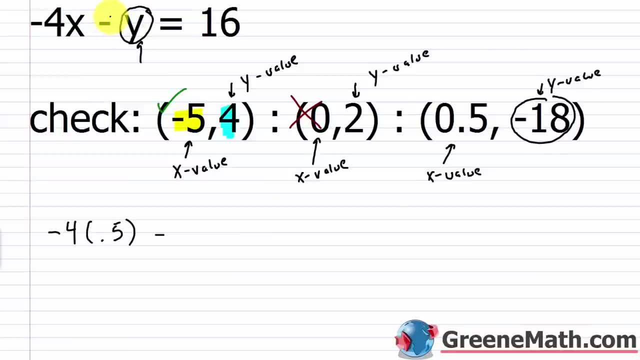 There's a minus sign already out in front. So this stays there. And then you put minus 18. Or negative 18. And minus a negative is plus a positive. So I can write minus 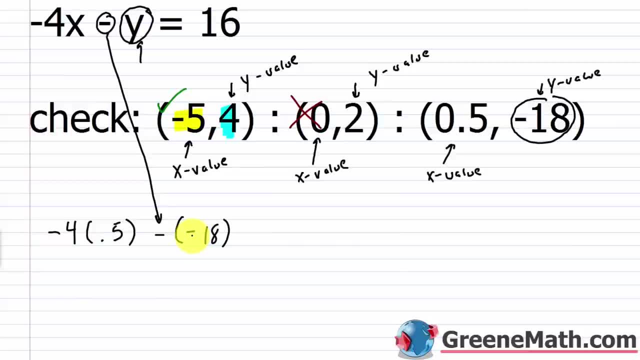 a negative 18. Or I could simplify that and put plus positive 18. Which I'm going to do in the next step. So equals 16. 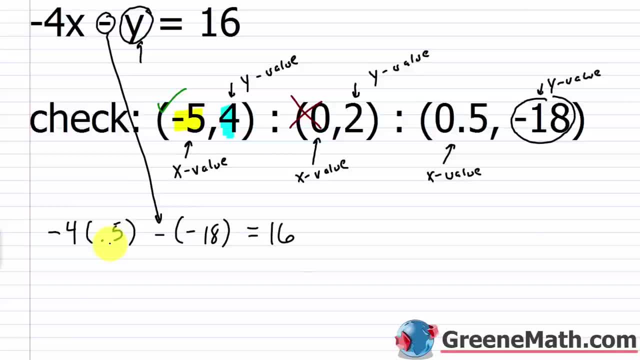 So what's negative 4 times 0.5? Again you could do that using negative 4 times 1 half. And kind of mentally say negative 4 times a half is negative 2. So this is negative 2. Minus a negative 18 is plus 18. 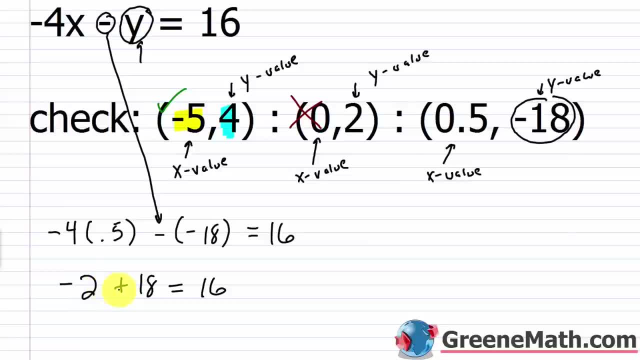 Equals 16. And so yeah this is going to be true. Negative 2 plus 18 is 16. 16 does equal 16. Same value on each side of the equation. And so we're going to check mark this and say yes. It is a solution to the equation. 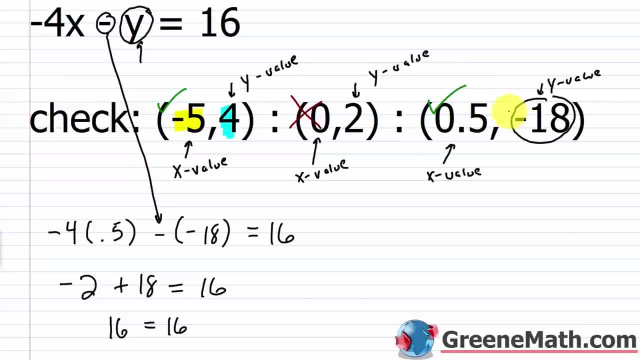 And one thing this would immediately draw your attention to is the fact that we can have more than one ordered pair that works as a solution to a linear equation in two variables. 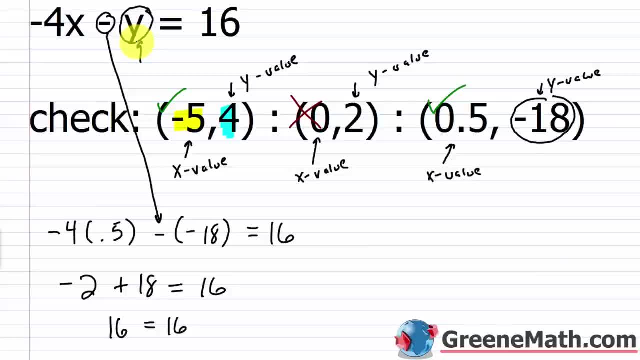 When we worked with a linear equation in one variable, generally speaking we're going to have exactly one value for our variable that makes the equation true. Here we have multiple ordered pairs or multiple solutions here that work. And in fact you're going to find that with a linear equation in two variables 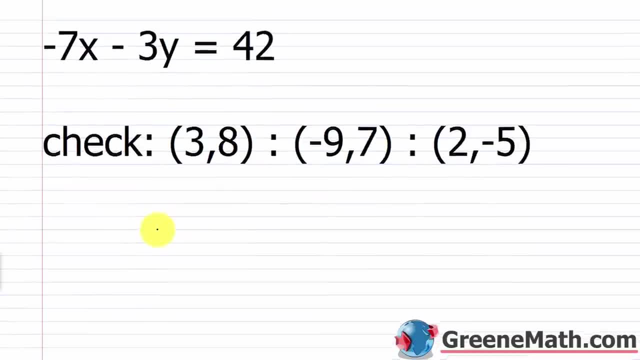 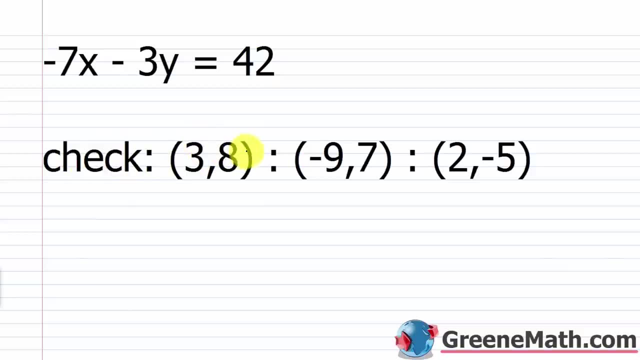 there's an infinite number of ordered pair solutions. Alright so now we're going to look at negative 7x minus 3y equals 42. And we want to check the ordered pair 3 comma 8. The ordered pair negative 9 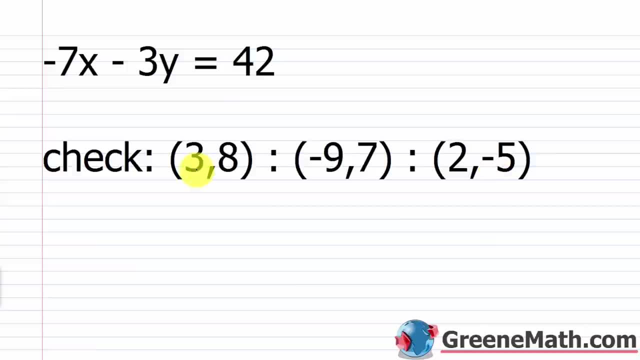 comma 7 and the ordered pair 2 comma negative 5. So let's start 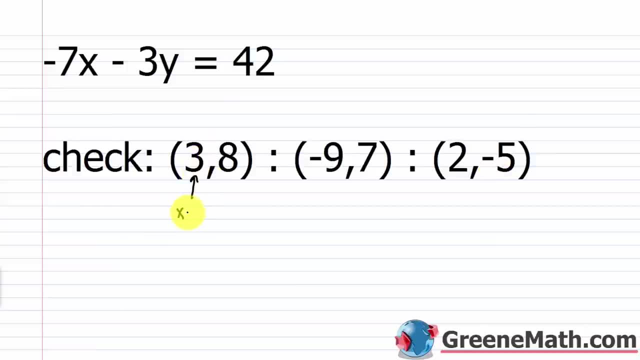 with this ordered pair 3 comma 8. So this is your x value. This is your y value. 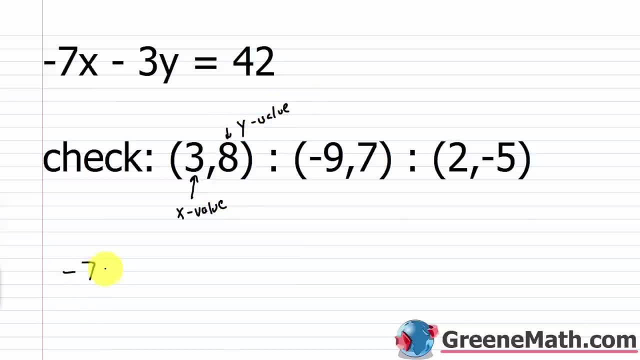 And let's do some plugging in. So we have negative 7 times for my x value I'm putting in a 3 minus 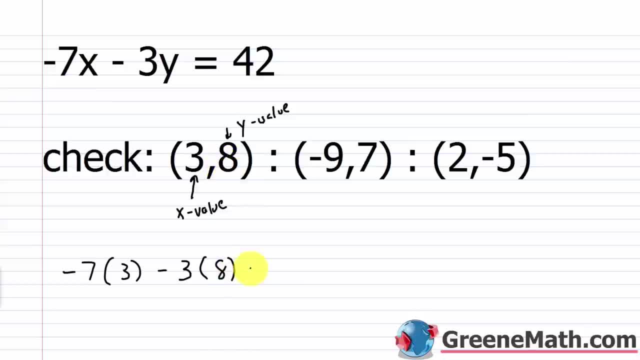 3 times for my y value I'm putting in an 8. 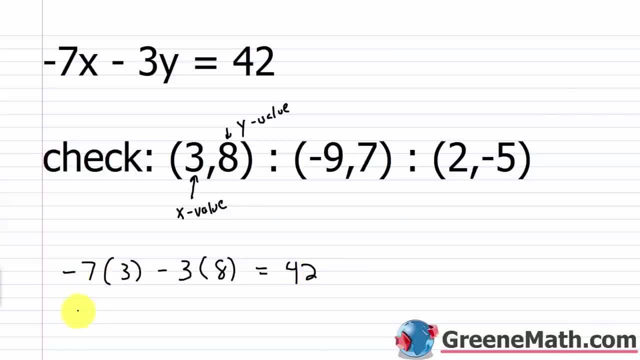 And this should be equal to 42. Negative 7 times 3 is negative 21. 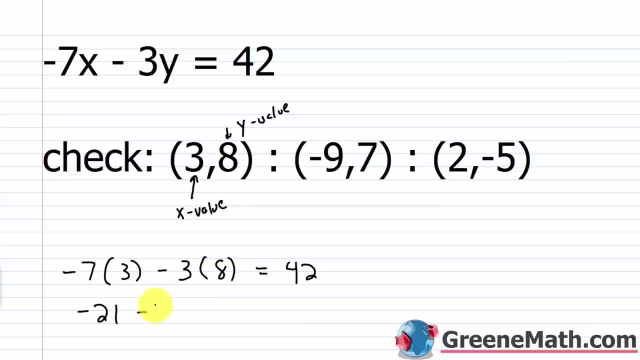 Negative 3 times 8 is negative 24. So minus 24 equals 42. 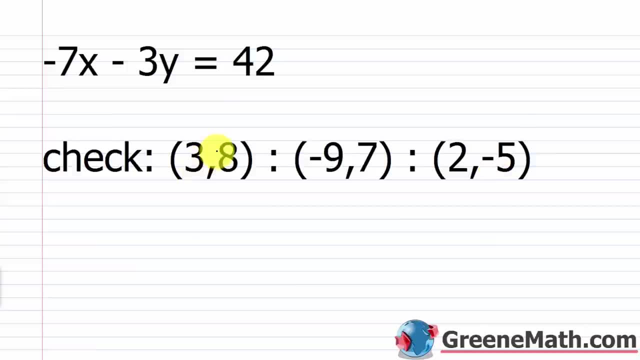 the ordered pair 2, comma negative 5. so let's start with this. ordered pair 3, comma 8. so this is your x value, this is your y value and let's do some plugging in. so we have negative 7 times for my x value. i'm putting in a 3 minus 3 times for my y value. i'm putting in an 8. 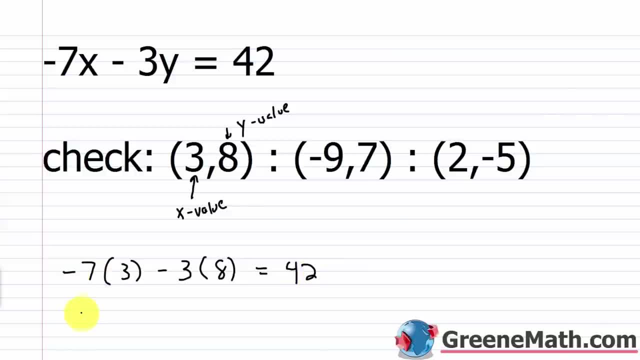 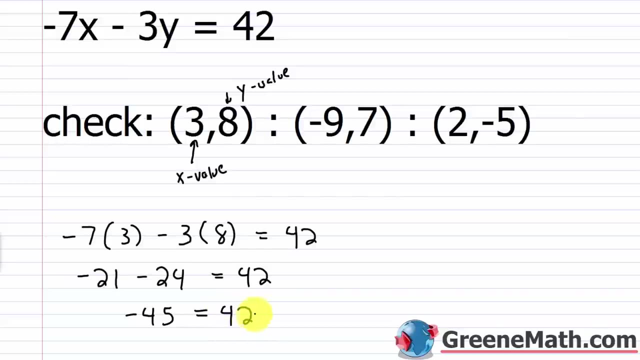 and this should be equal to 42. negative 7 times 3 is negative 21. negative 3 times 8 is negative 24. so minus 24 equals 42. negative 21 minus 24 is negative 45 and this is not equal to 42. this is false. 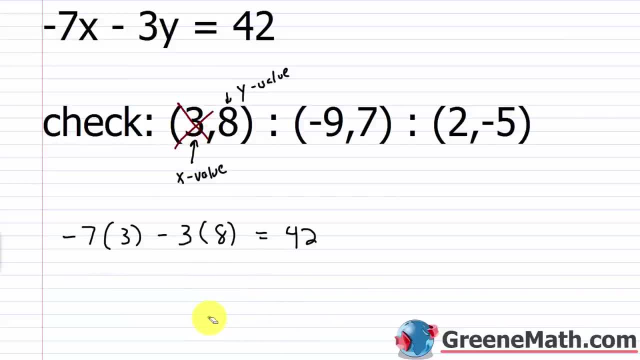 so this does not work out as a solution. to make this a little quicker, i'm just gonna- i'm just gonna- erase this part, which is where we plugged in right, the rest of the equation is always going to be the same. you'll have your taxes right here. the rest of the equations always going to be the same. 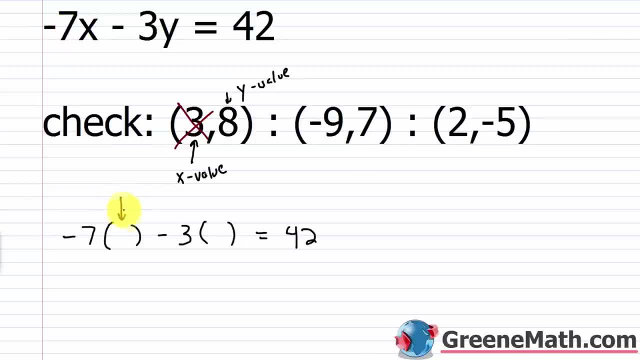 you'll have your negative 7 times your spot for x, then minus 3 times your spot for y, then equals 42. so I'm just going to erase those parts. now I'm going to be plugging in a negative 9 for x. this is my x value, so negative 9 goes here. right, we have negative 7 times x, so negative 7 times. 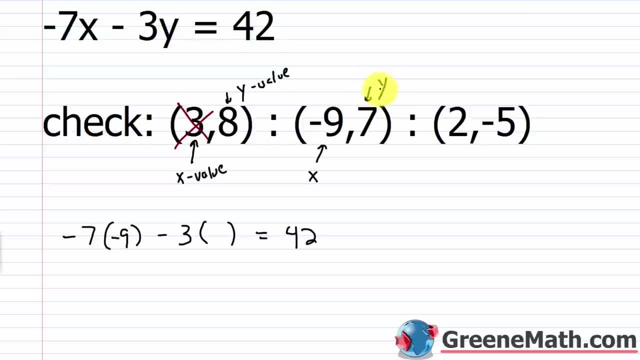 negative 9 and I'm going to plug in a 7 for y again. here's my y value: I have negative 3 times y, so I'm plugging in a 7 for y, so I go negative 3 times 7. so negative, 7 times negative, 9 minus. 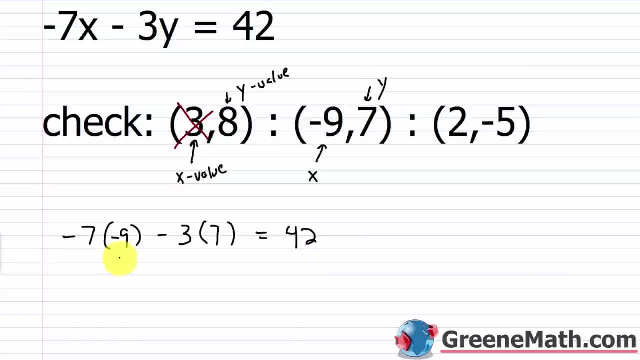 3 times 7 equals 42. negative 7 times negative: 9 is 63 minus 3 times 7 is 21. this should equal 42 and in fact it does. 63 minus 21 is 42. so you get 42 equals 42. that checks out. 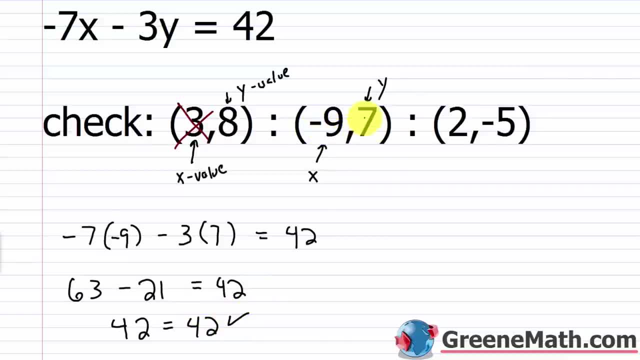 and so we can say that negative 9 comma 7, this ordered pair, is a solution. all right, let's do one more and again. I'm just going to erase the part where we plug in and I have a 2 that's going to represent my x value and a negative 5 that's going to represent my y value. 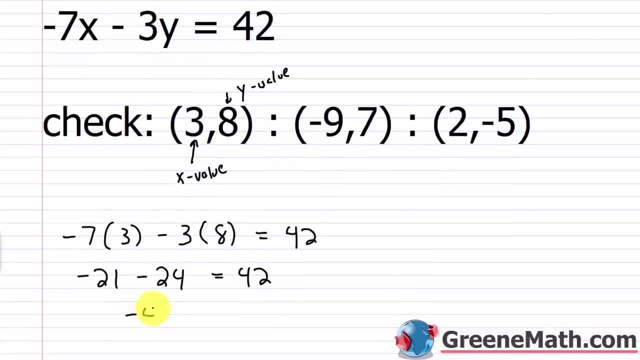 Negative 21 minus 24 is negative 45. 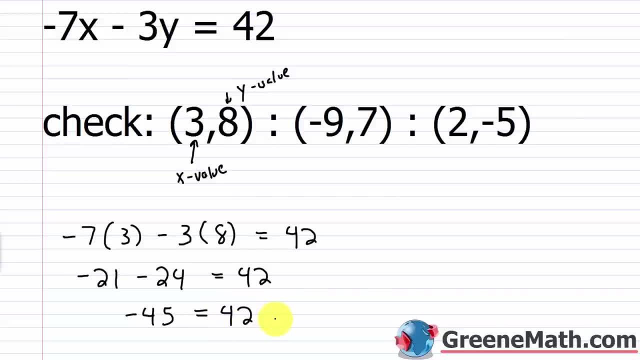 And this is not equal to 42. This is false. So 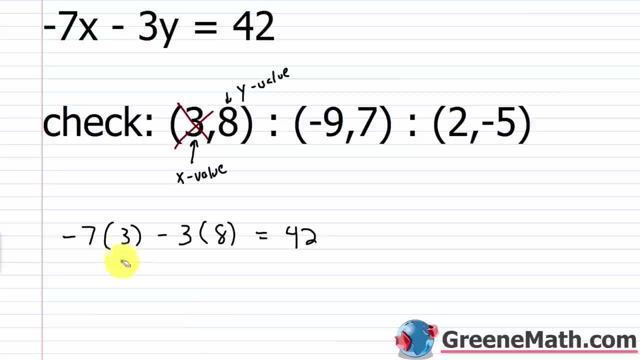 this does not work out as a solution. To make this a little quicker I'm just going to erase this part which is where we plugged in. The rest of the equation is always going to be the same. You'll have your negative 7 times your spot for x then minus 3 times your spot for y then equals 42. So I'm just going to erase those parts. 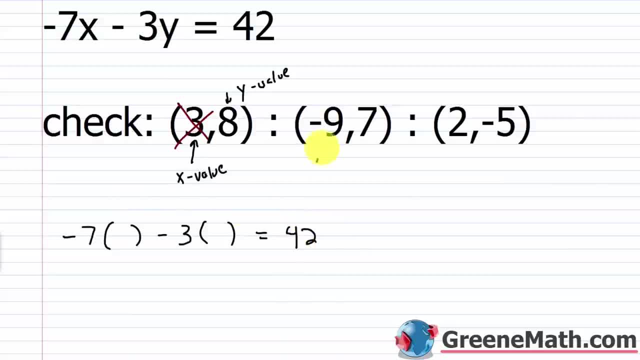 Now I'm going to be plugging in a negative 9 for x. This is my x value. So negative 9 goes here. We have negative 7 times x. So negative 7 times negative 9. And I'm going to plug in a 7 for y. Again, here's my y value. I have negative 3 times y. So I'm plugging in a 7 for y. So I go negative 3 times 7. So negative 7 times negative 9 minus 3 times 7 equals 42. 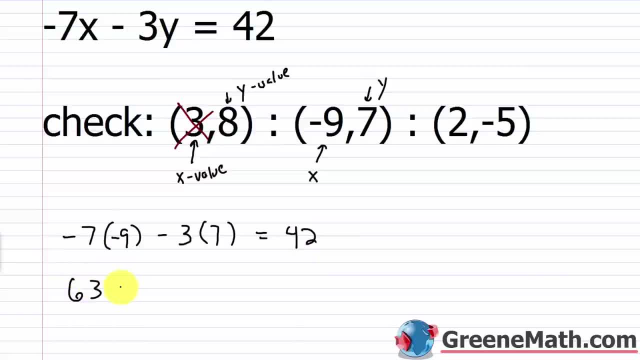 Negative 7 times negative 9 is 63. Minus 3 times 7 is 21. This should equal 42. And in fact it does. 63 minus 21 is 42. So you get 42 equals 42. 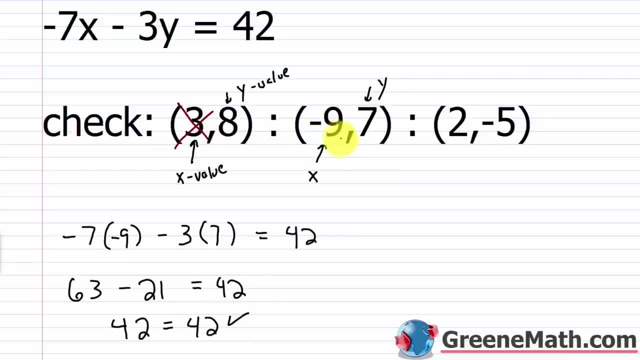 That checks out. And so we can say that negative 9 comma 7, this ordered pair, is a solution. Alright let's do one more. 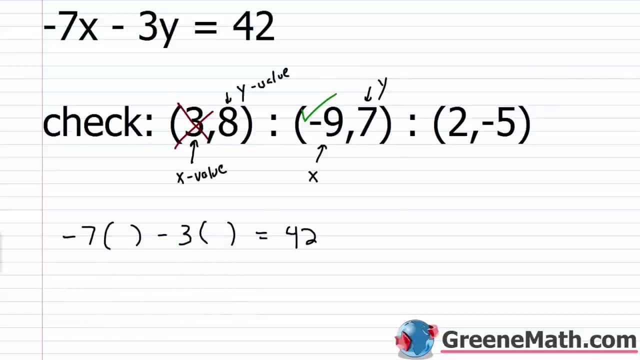 And again I'm just going to erase the part where we plug in. And I have a 2 that's going to represent my x value. And a negative 5 that's going to represent my y value now. So where's x? We have negative 7 times x. Negative 7 times this right here. So 2, which is my value for x, is going to go in right here. And then my y value of negative 5 is going to go in right here. Alright again I'm just plugging it in right there next to negative 3. So I have negative 7 times 2 minus 3 times negative 5 equals 42. 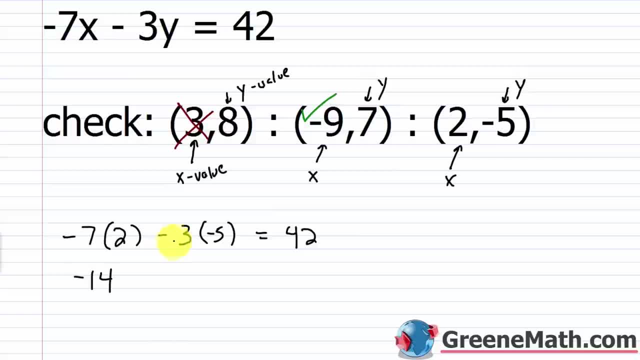 Negative 7 times 2 is negative 14. Negative 3 times negative 5 is 15. So plus 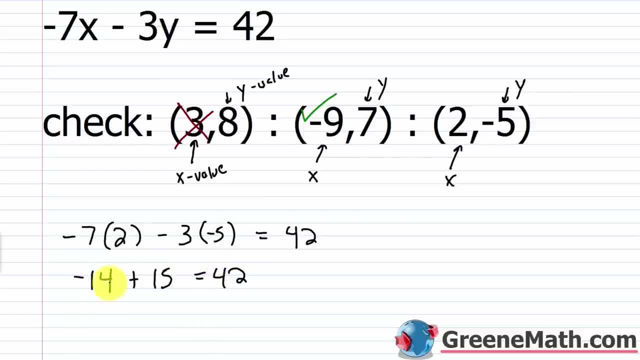 15 equals 42. Negative 14 plus 15 is 1. And 1 is not equal to 42. This is false. 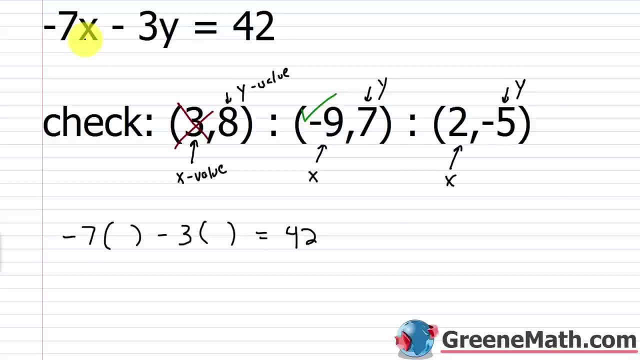 now. so where's x? we have negative 7 times x, negative 7 times this, right here. so 2, which is my value for x, is going to go in right here, and then my y value of negative 5 is going to go in right here, right again. I'm just plugging it in right there, next to negative 3, so I have negative. 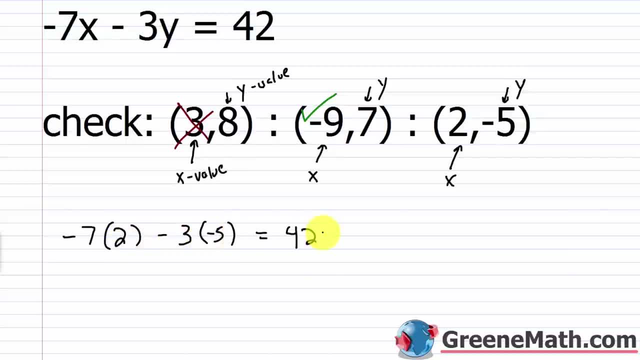 7 times 2 minus 3 times negative 5 equals 42. negative 7 times 2 is negative. 14. negative 3 times negative, 5 is 15. so plus 15 equals 42. negative 14 plus 15 is 1 and 1 is not equal to 42. this is false, so this doesn't work out. 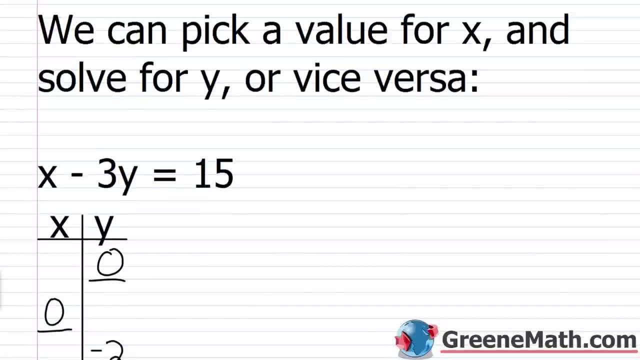 so for these type of equations, we can pick a value for x and solve for y, or vice versa. so I could pick a value for y and solve for y, so I could pick a value for y and solve for y, so I could pick a value for x. and this is going to be a very important skill that we're going to use. 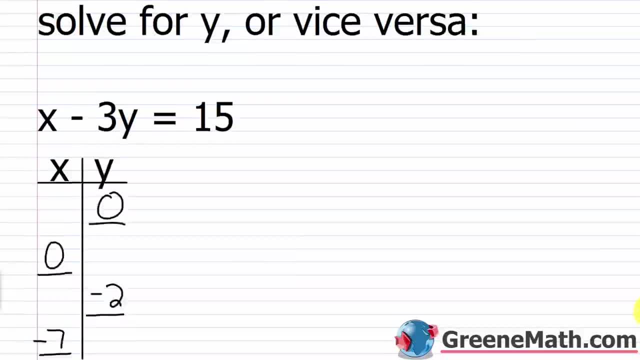 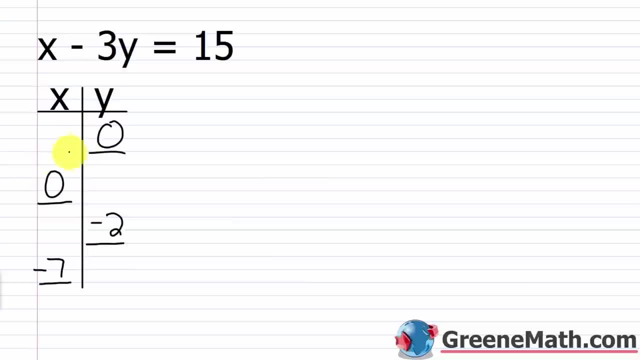 throughout this chapter. all right, so let's start out by looking at this equation. we have x minus 3y equals 15. now I'm given some values for x and for y here. this is a table of values, and what's going to happen is okay. for example, here I'm given a value of 0, so I would plug 0 in for y. 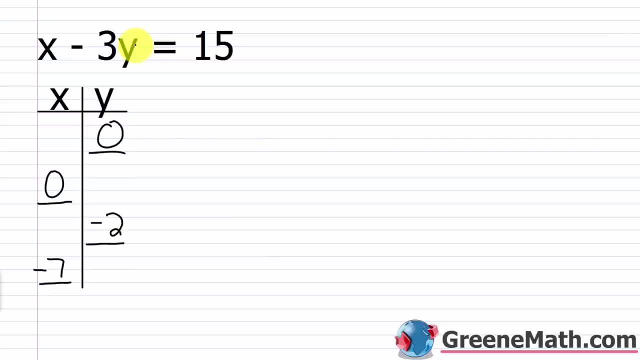 and I would solve for x. so let me show you what that looks like. so we have x minus 3 times y. I have a given value of 0 for y, so I'm going to plug that in equals 15. so then, if I simplify this, I'd have x equals 15. 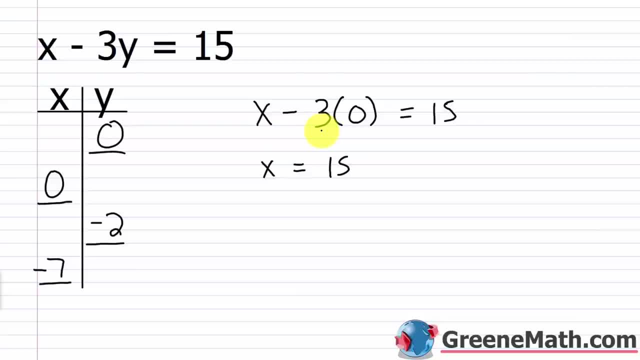 right. 3 times 0 is just 0. if I'm subtracting away 0, it's like I just have x. all right, so x equals 15, so that's the value for x. that makes this equation true when y is 0. so I can go ahead. 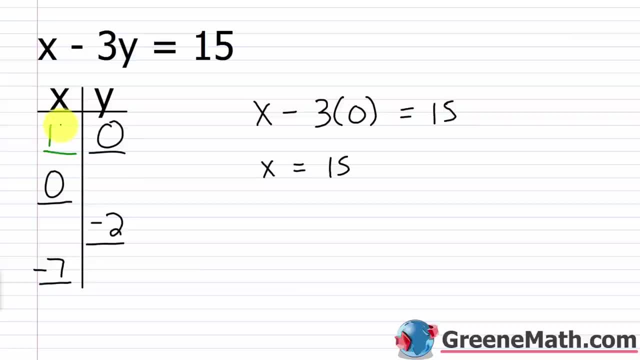 and fill in the missing value and put: okay, this is 15. so the ordered pair. the ordered pair 15, comma 0 is a solution to this equation. right, 15 is my value for x. the value on the left. 0 is my value for y, the value on the right. all right, so now I'm given an x value of 0. So this doesn't work out. 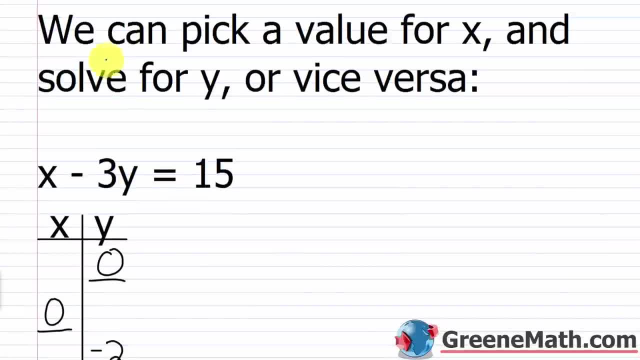 So for these type of equations, we can pick a value for x and solve for y or vice versa. 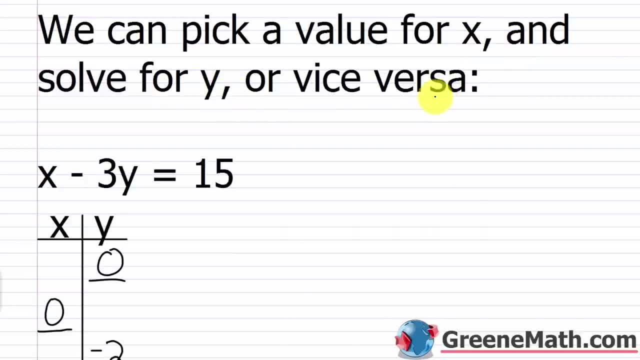 So I could pick a value for y and solve for x. And this is going to be a very important skill that we're going to use throughout this chapter. 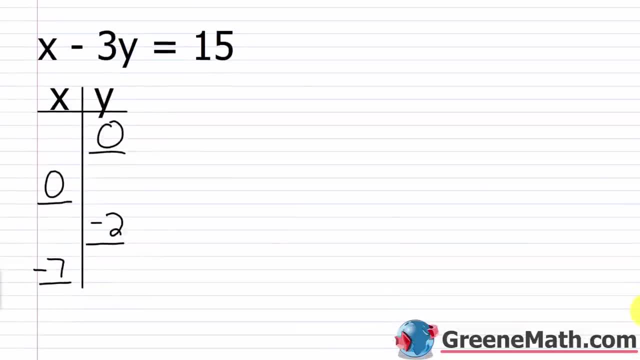 Alright so let's start out by looking at this equation. 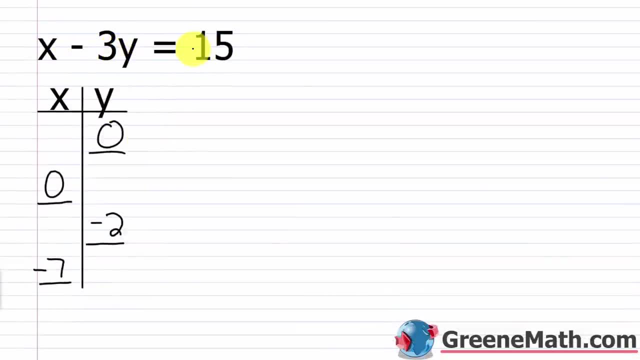 We have x minus 3y equals 15. 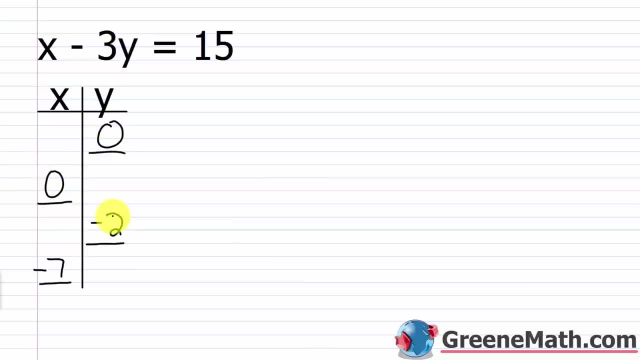 Now I'm given some values for x and for y here. This is a table of values. 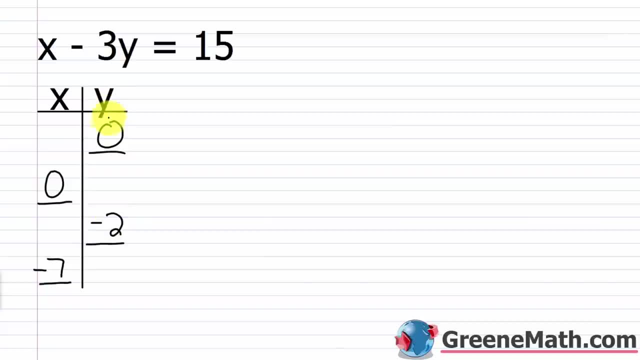 And what's going to happen is, for example here, I'm given a value of 0. So I would plug 0 in for y and I would solve for x. 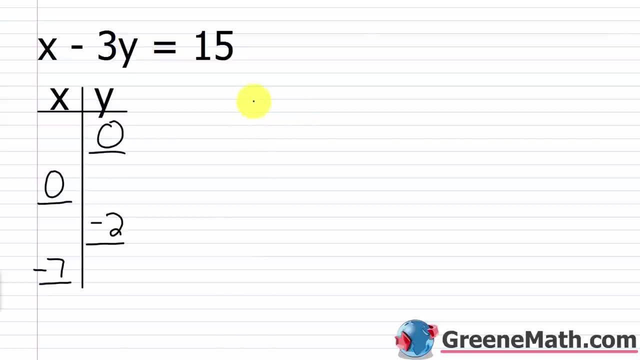 So let me show you what that looks like. So we have x minus 3 times y. I have a given value of 0 for y so I'm going to plug that in. equals 15. So then, if I simplify this, I'd have x equals 15. Right? 3 times 0 is just 0. If I'm subtracting away 0, it's like I just have x. 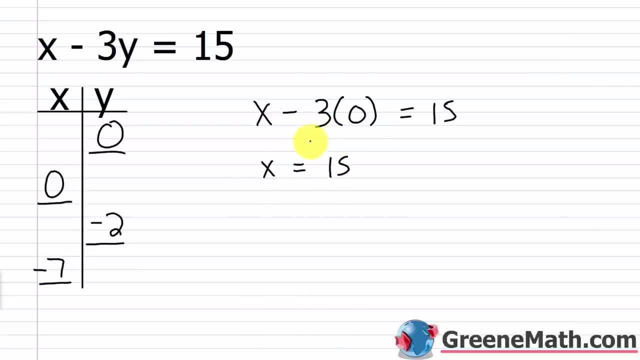 Alright so x equals 15. So that's the value for x that makes this equation true when y is 0. So I can go ahead and just fill in the missing value and put, okay this is 15. So the ordered pair 15 comma 0 is a solution to this equation. 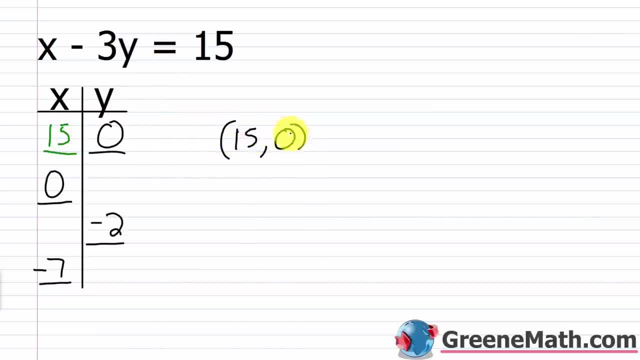 Right? 15 is my value for x, the value on the left. 0 is my value for y, the value on the right. Alright so now I'm given an x value of 0. So I'm going to plug a 0 in for x. So instead of x minus 3y equals 15 I'm going to put 0 minus 3y equals 15. 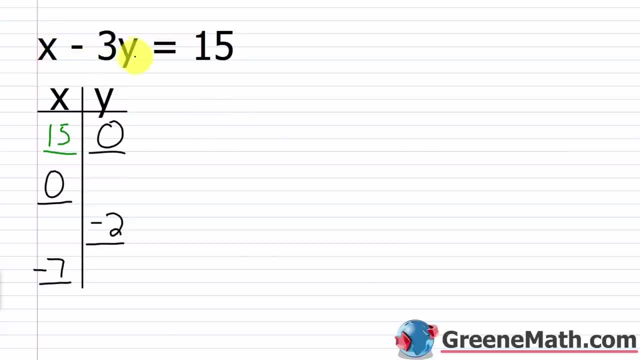 so I'm going to plug a 0 in for x. so instead of x minus 3y equals 15, I'm going to put 0 in, for y equals 15. really, the 0 out in front doesn't do anything, so I can just get rid of it. 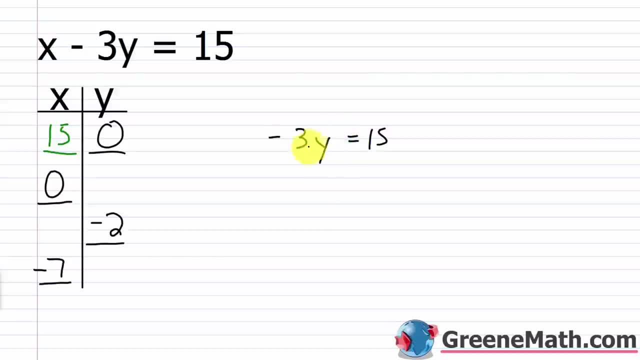 and I'm left with negative 3y equals 15. so to solve for y- we already know how to do that. I want to isolate y, so I just divide both sides of the equation by negative 3, nothing we haven't done before. this will cancel with this and I'll just have y, and then it equals 15 divided by. 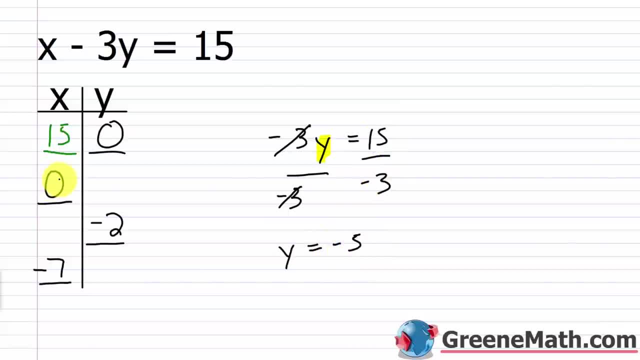 negative 3 is negative 5. so if x is 0, y equals negative 5. let me kind of put that in a different color so it stands out. so let's put negative 5 here. so again, this is another ordered pair that works as a solution to this equation. 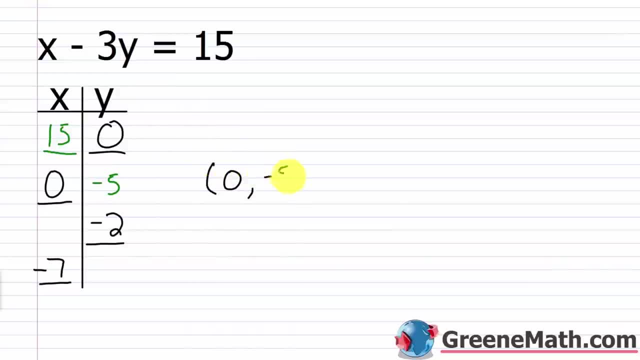 we can put the ordered pair 0 comma. negative 5 is a solution again, where 0 is the x value and negative 5 is the y value. right now we're given a y value of negative 2. we want to find the missing x value, so we have x minus. I'm plugging in a negative 2 for y, so I'm going to. 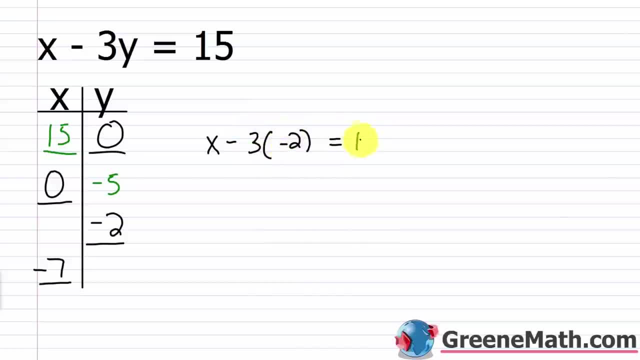 have 3 times negative 2 equals 15.. So negative 3 times negative 2 is 6. so I would really have x plus 6 equals 15, and I want to solve for x and again, we know how to do that. if we want x by itself, I just need to. 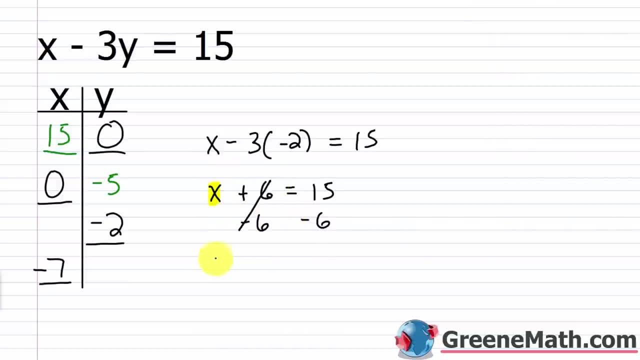 subtract 6 away from each side of the equation, so that's going to cancel. I'm going to have: x is equal to 15 minus 6 is 9, so x equals 9, so let's put that over here, and I'm going to remember to use a different color this time and I'm going to put 9 there, so that's. 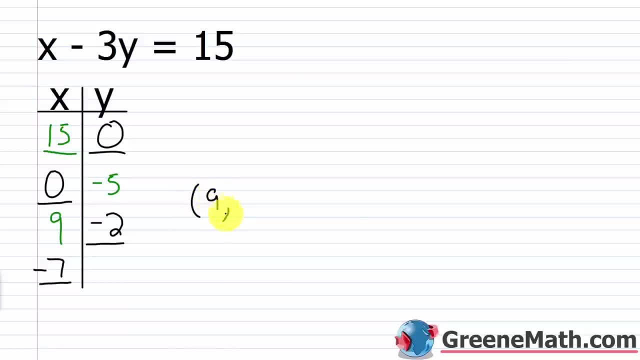 an ordered pair that works as a solution. so we can say: the ordered pair 9, comma negative 2 again works as a solution for this equation. Let's do one more. we're given an x value of negative 7, so I'd plug a negative 7 in for. 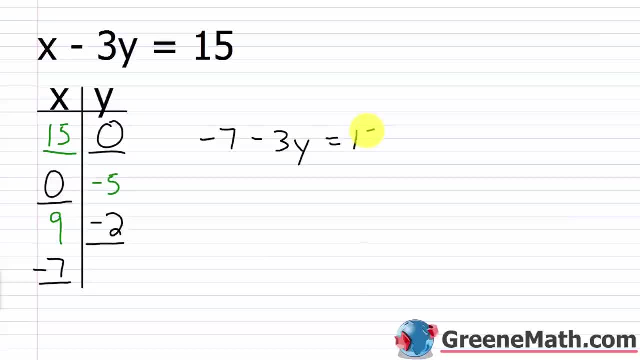 x. so then minus 3y equals 15. I want y by itself, so I'm going to add 7 to each side of the equation. that's gone, I'll have negative. 3y is equal to 22 if I divide both sides of the. 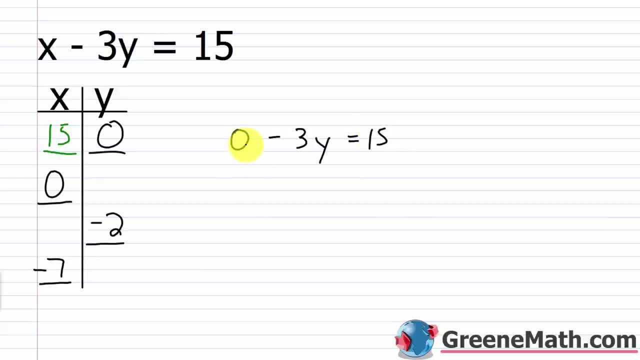 Really, the 0 out in front doesn't do anything so I can just get rid of it. And I'm left with negative 3y equals 15. So to solve for y, we already know how to do that. I want to isolate y. So I just divide both sides of the equation by negative 3. Nothing we haven't done before. This will cancel with this and I'll just have y. 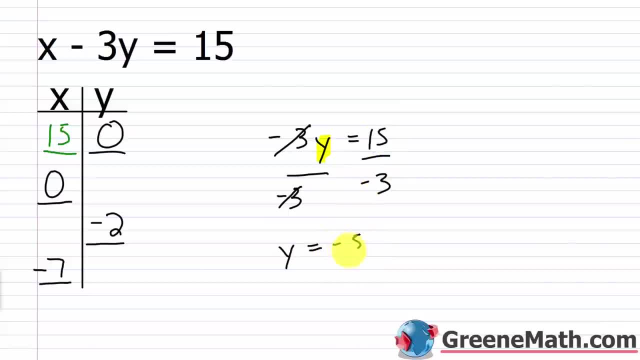 And then it equals 15 divided by negative 3 is negative 5. 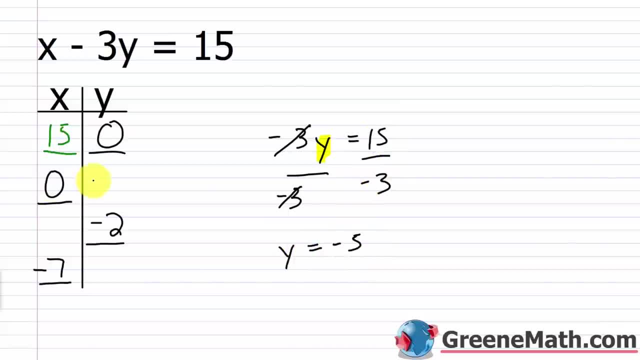 So if x is 0, y equals negative 5. 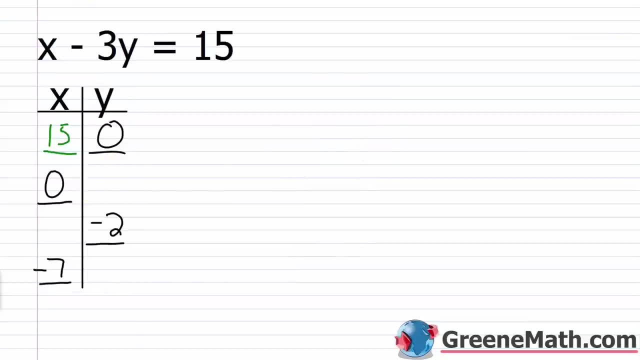 Let me kind of put that in a different color so it stands out. So let's put negative 5 here. So again, this is another ordered pair that works as a solution to this equation. 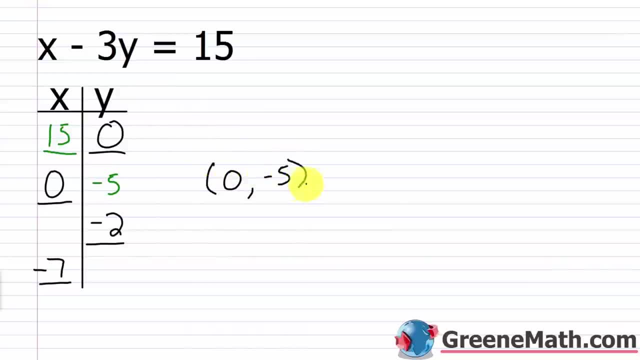 We can put the ordered pair 0 comma negative 5 is a solution. 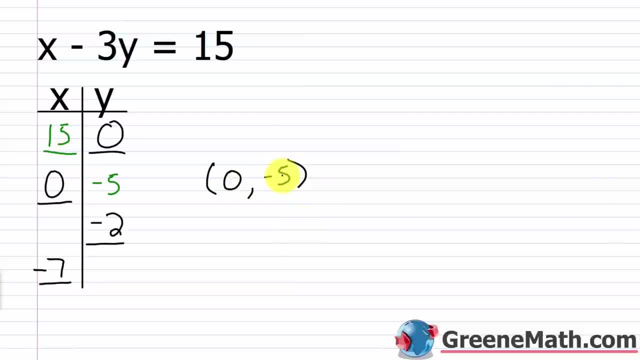 Again, where 0 is the x value and negative 5 is the y value. 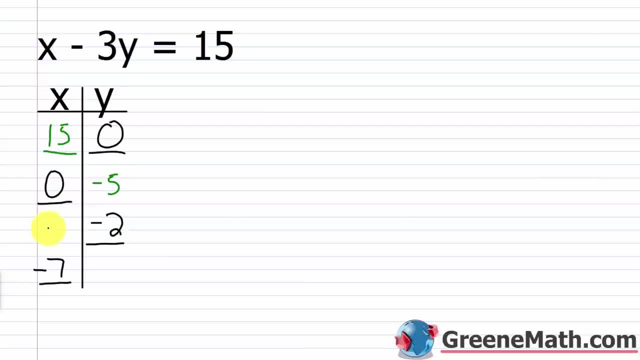 Alright, now we're given a y value of negative 2 and we want to find the missing x value. So we have 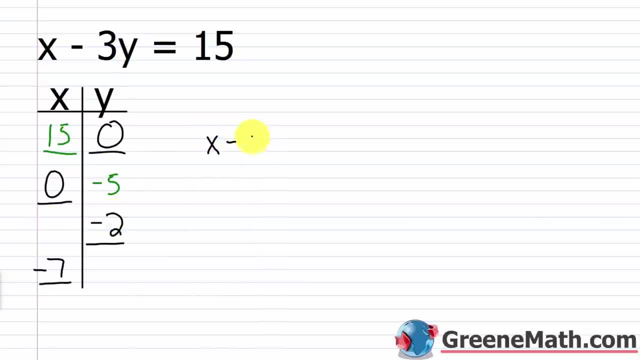 x minus, I'm plugging in a negative 2 for y. So I'm going to have 3 times negative 2 equals 15. 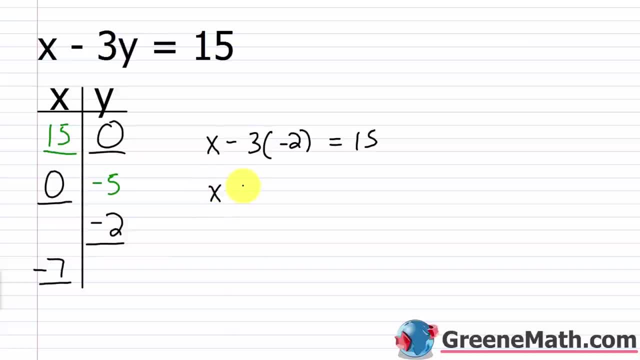 So negative 3 times negative 2 is 6. So I would really have x plus 6 equals 15. 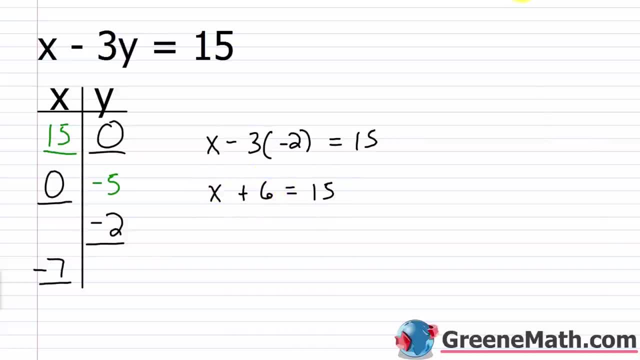 And I want to solve for x. And again, we know how to do that. If we want x by itself, I just need to subtract 6 away from each side of the equation. So that's going to cancel. I'm going to have x is equal to 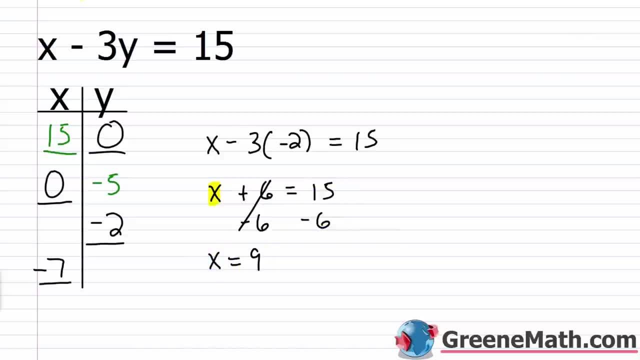 15 minus 6 is 9. So x equals 9. So let's put that over here. 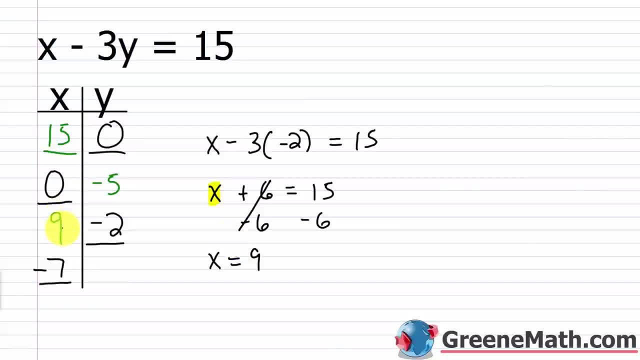 And I'm going to remember to use a different color this time. And I'm going to put 9 there. 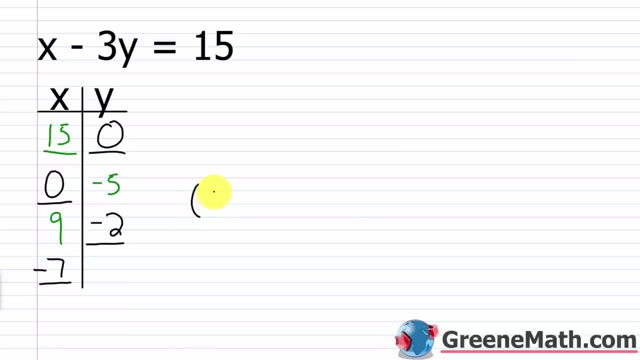 So that's another ordered pair that works as a solution. So we can say the ordered pair 9 comma negative 2, again works as a solution for this equation. 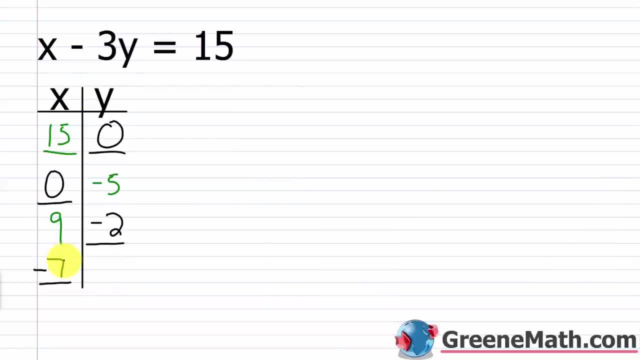 Now let's do one more. We're given an x value of negative 7. 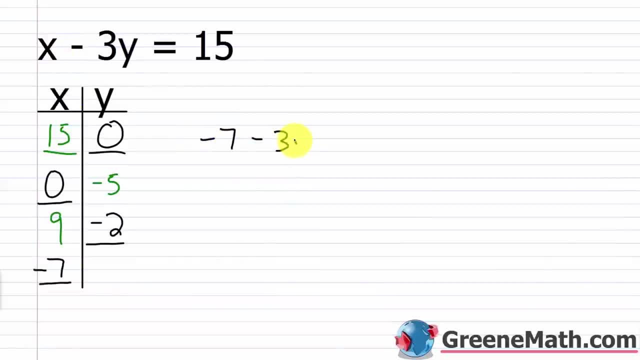 So I'd plug a negative 7 in for x. So then minus 3y equals 15. I want y by itself, so I'm going to add 7 to each 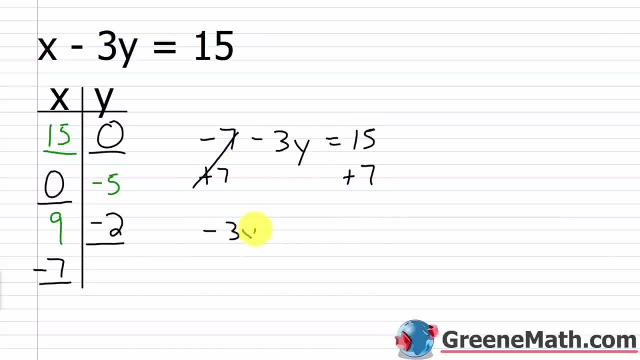 side of the equation. That's gone. I'll have negative 3y is equal to 22. 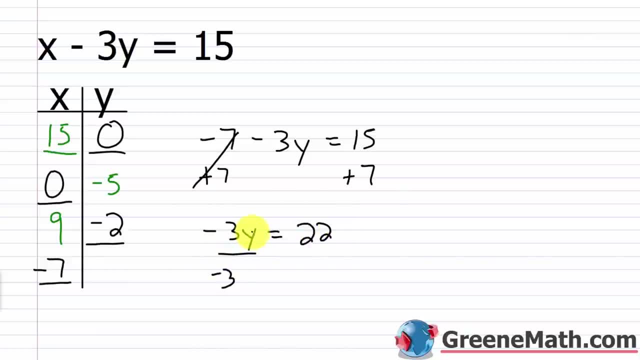 If I divide both sides of the equation by negative 3, so that y can be by itself, this will cancel with this. And I'll have y equals negative 22 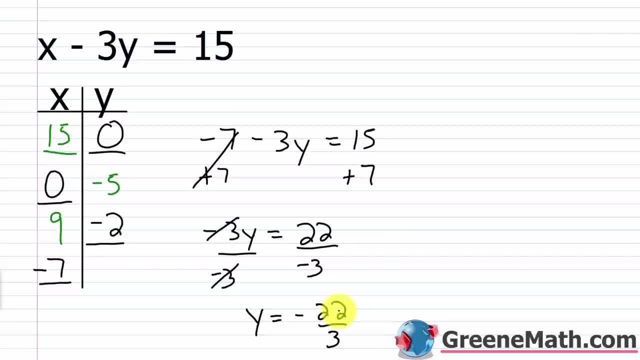 thirds. And there's nothing to do to simplify that. 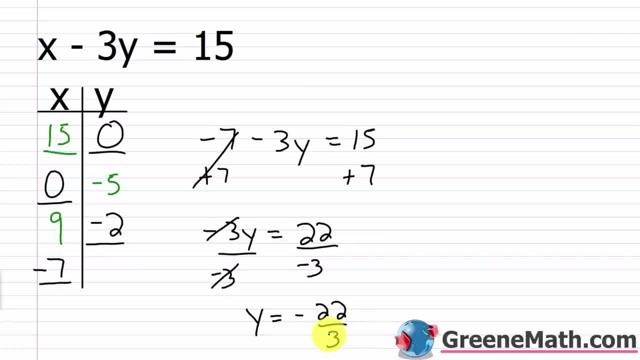 22 is 11 times 2. I can't really cancel anything with the 3. We'll write that 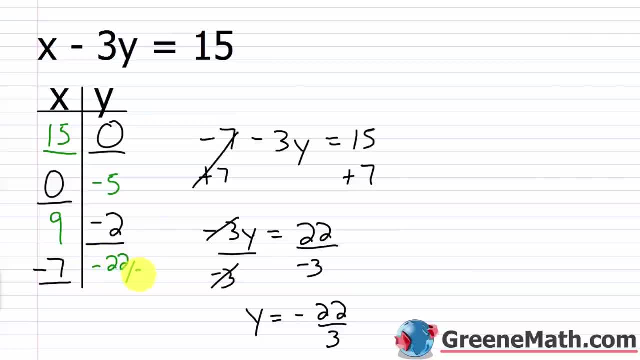 over here as negative 22 thirds. 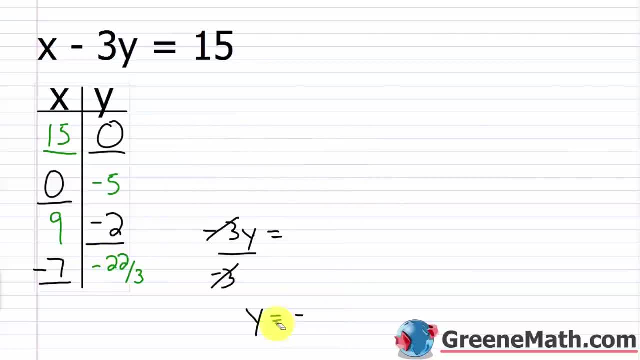 And again, that's another ordered pair that's a solution to our equation. Let's just write that real quick. 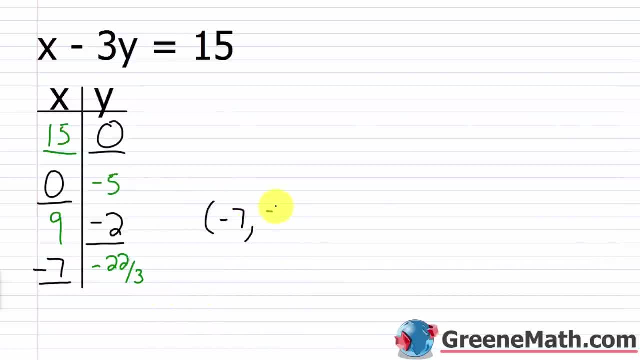 It would be negative 7 comma negative 22 thirds. 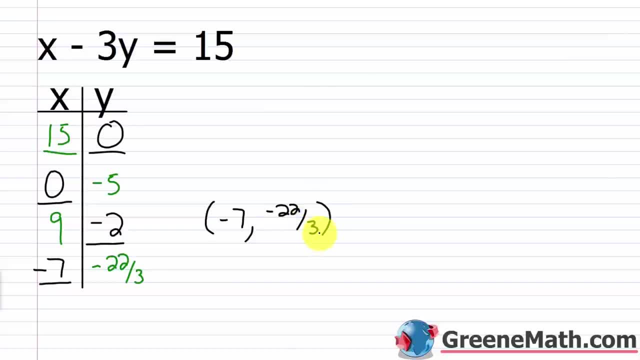 And I can go through and keep generating as many ordered pair solutions as I want. I can pick a value for x. Doesn't matter what it is. I can plug it in and I can solve for y. So that would give me the x value that I picked and the y value that I solved for. Put those two together, that gives me an ordered pair that's a solution. 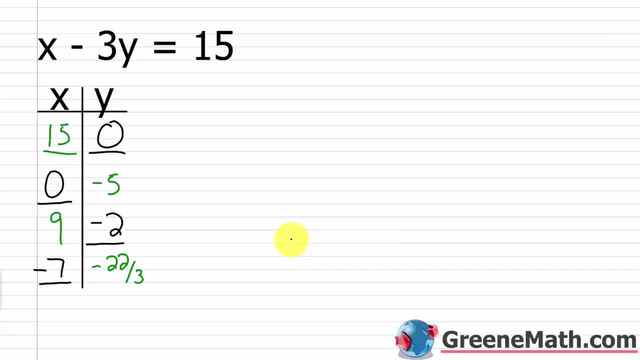 I could do the opposite thing. I could pick a value for y and solve for x. 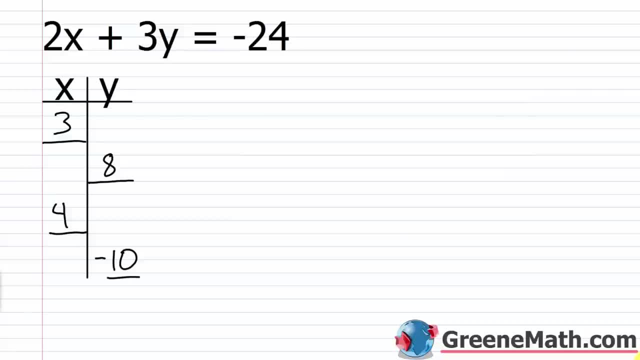 Alright, let's take a look at another example of this. So we have 2x plus 3y equals negative 24. So we're given an x value of 3. We want to solve for the unknown y value. So if x equals 3 here, I would have 2 times, I'm plugging in a 3 for x, plus 3y equals negative 24. 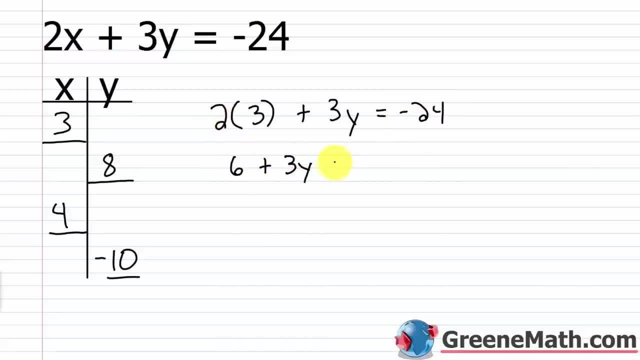 So 2 times 3 is 6. So I would have 6 plus 3y equals negative 24. 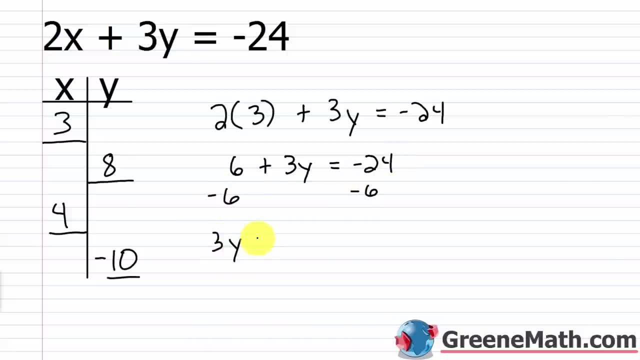 Subtract 6 away from each side. I'd have 3y equals negative 30. 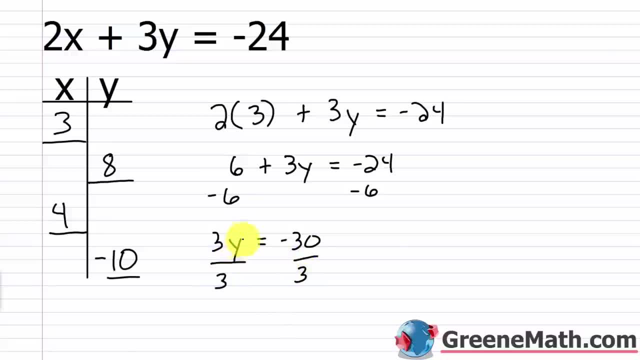 And then I would divide both sides by 3. Alright, in order to isolate the variable y. This cancels with this. 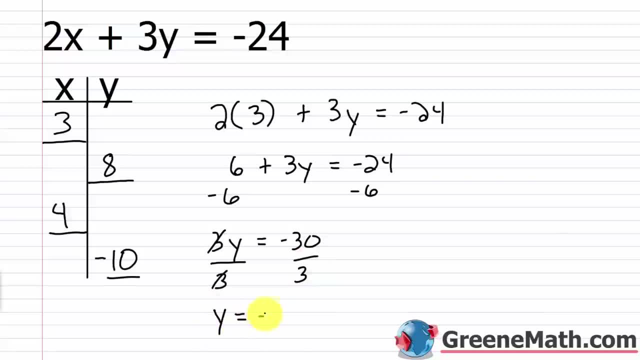 Negative 30 divided by 3 is negative 10. So you get y equals negative 10. So I can put a negative 10 there. And so my ordered pair would be 3 for my x value, comma negative 10 for my y value. Now let's look at 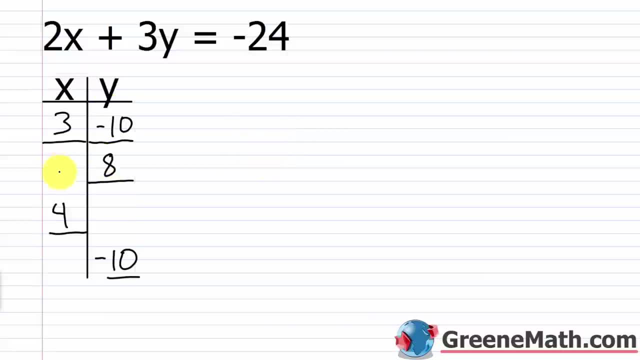 we're given a y value of 8. We want to find the unknown x value. So we have 2x plus 3. 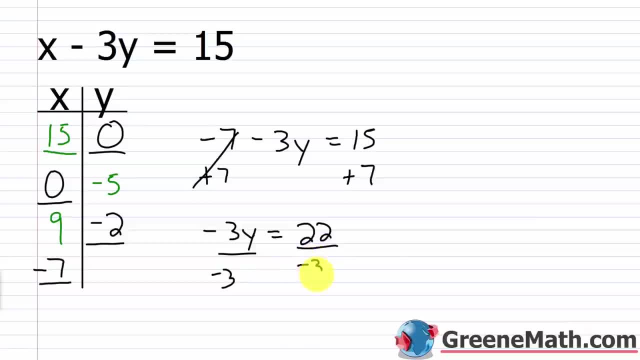 equation by negative 3 so that y can be by itself. This will cancel with this and I'll have y equals negative 22 thirds and there's nothing to do. to simplify that: 22 is 11 times 2. I can't really cancel anything with the 3 we'll. 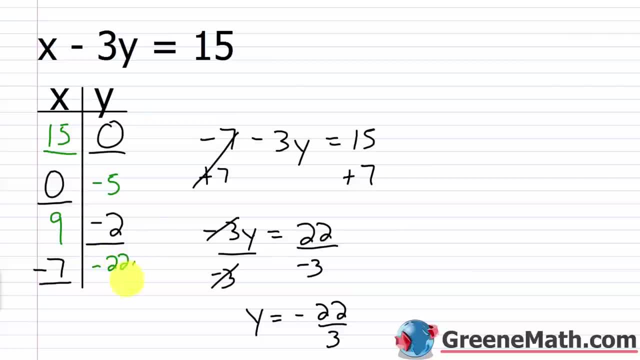 write that over here as negative 22 thirds and again, that's another ordered pair. that's a solution to our equation. let's just write that real quick. it would be negative 7 comma, negative 22 thirds, And I can go through that. I can go through and keep generating as many ordered pair solutions as I want. I can pick. 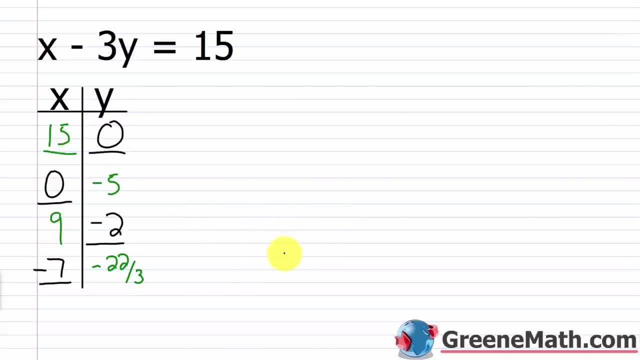 a value for x, doesn't matter what it is, I can plug it in and I can solve for y. so that would give me the x value that I picked and the y value that I solved for. put those two together. that gives me an ordered pair. that's a solution. I could do the opposite thing. I. 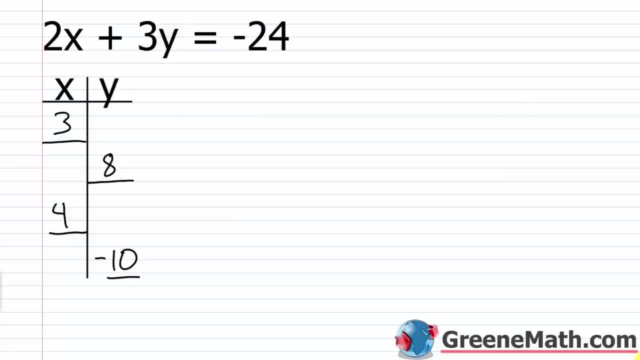 could pick a value for y and solve for x. Alright, let's take a look at another example of this. so we have 2x plus 3y equals negative 24.. So we're given an x value of 3. we want to solve for the unknown y value. so if x equals, 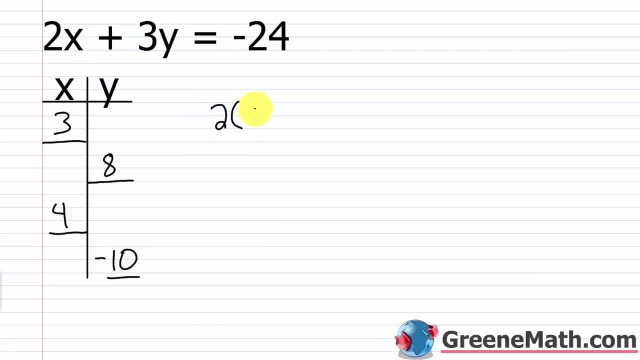 3 here, I would have 2 times- I'm plugging in a- 3- for x plus 3y equals negative 24, so 2 times 3 is 6, so I would have 6 plus 3y equals negative 24, subtract 6 away from each side. 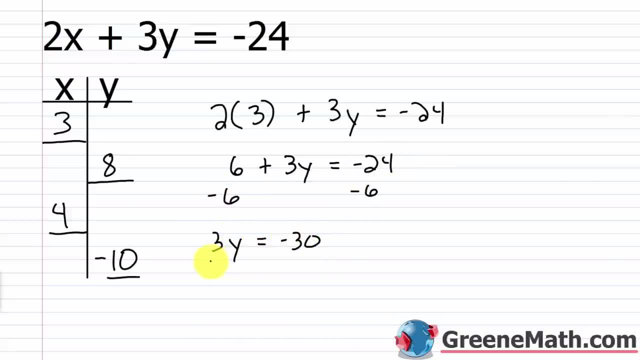 I'd have 3y equals negative 30 and then I would divide both sides by 3.. Alright, looking for an x value in the order to isolate the variable y. This cancels with this: negative 30 divided by 3 is negative 10, so you get y equals negative. 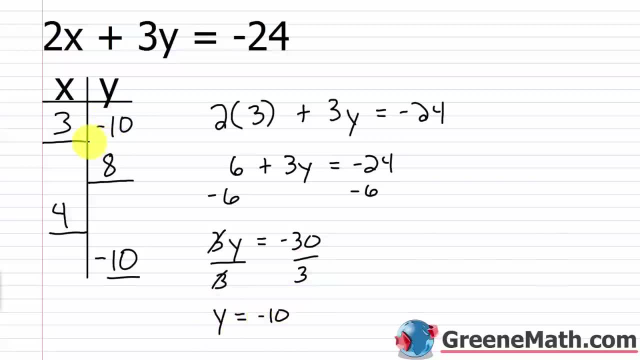 10, so I can put a negative 10 there, and so my ordered pair would be 3 for my x value comma, negative 10 for my y value. Now we're given a y value of 8. we want to find the unknown x value, so we have 2x plus. 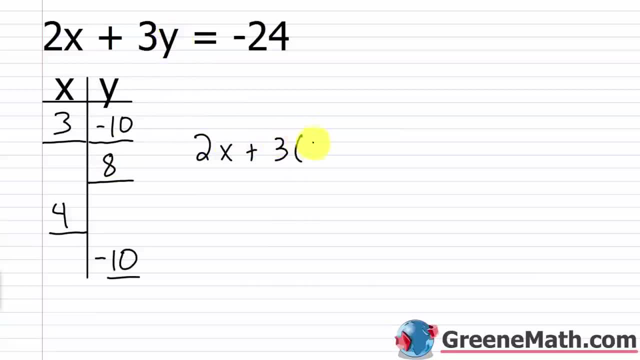 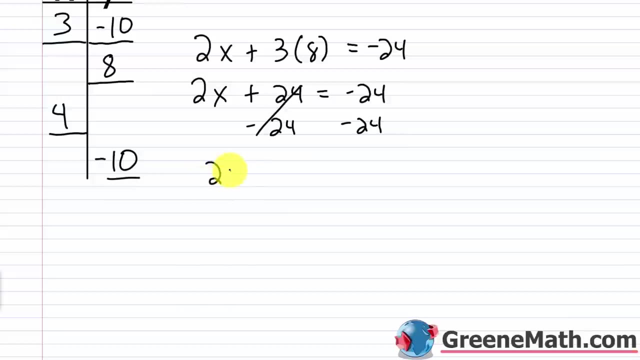 3. we're plugging in an 8 for y. this equals negative 24. so we have 2x plus 3 times 8 is 24 equals negative 24. we subtract 24 away from each side, that's going to cancel and i'm going to have 2x is equal to negative 24 minus. 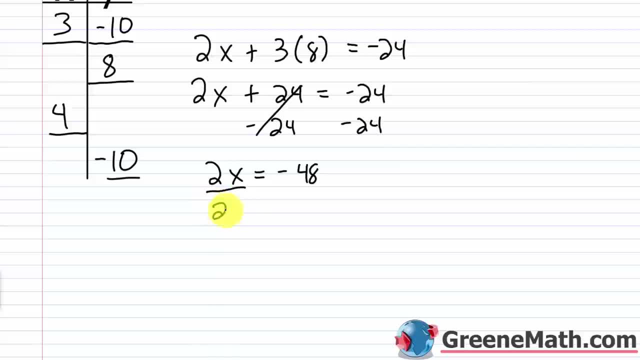 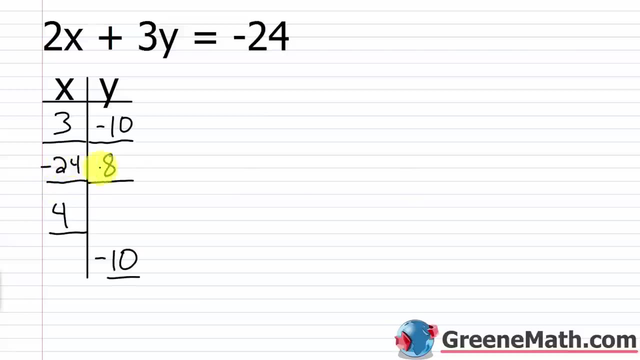 24 is negative 48. so now i can divide both sides of the equation by 2 in order to isolate x. this will cancel with this and i have: x is equal to negative 48 divided by 2 is negative 24. so we can come back up here and say that the missing value here is negative 24. right, this would be another. 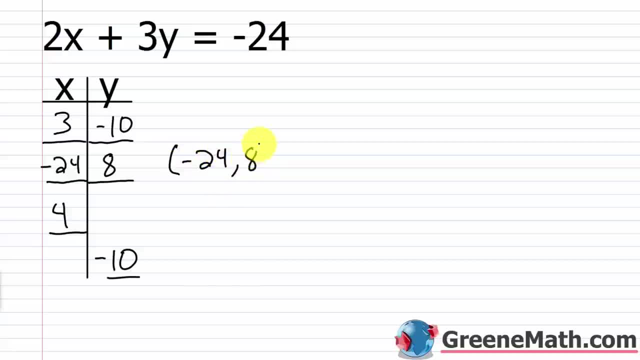 ordered pair solution: negative 24 for the x value, 8 for the y value. all right, for the next one, i have an x value of 4 and i want to find the unknown y value. so i'll have 2 times i have x. i'm plugging in a: 4 for x plus 3y equals negative 24. so 2 times 4 is 8, so we have 8 plus 3y. 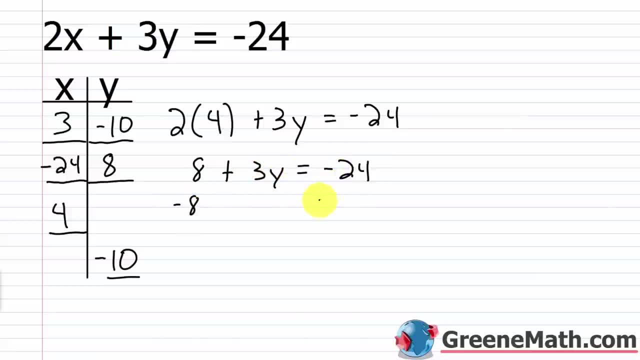 equals negative 24. we subtract 8 away from each side, we'll have 3y is equal to negative 32. divide both sides of the equation by 3 so that i can isolate y and i'll have: y is equal to negative 32 thirds and there's. 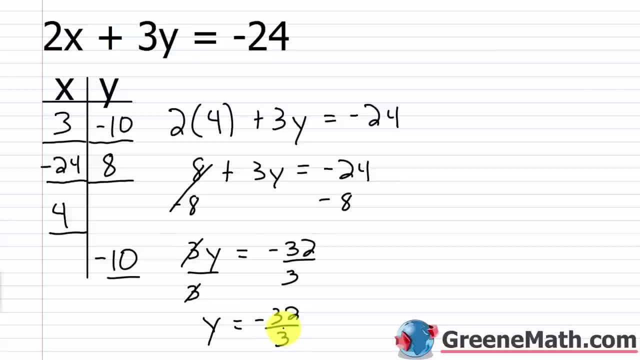 nothing i can do to simplify that. if i think about 32, that's 2 to the 5th power, right? i can't cancel any of those factors of 2 with this 3 here. so this is simplified. so our missing value for y would be negative 32 thirds. all right, so my ordered pair solution. 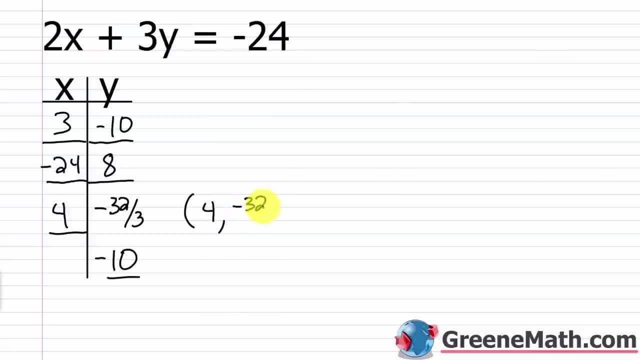 there would be 4 comma, negative 32 thirds. all right, for the last one we're going to look at, we're given a y value of negative 10, so we have 2x plus 3 times. i'm plugging in a negative 10 for y. We're plugging in an 8 for y. This equals negative 24. 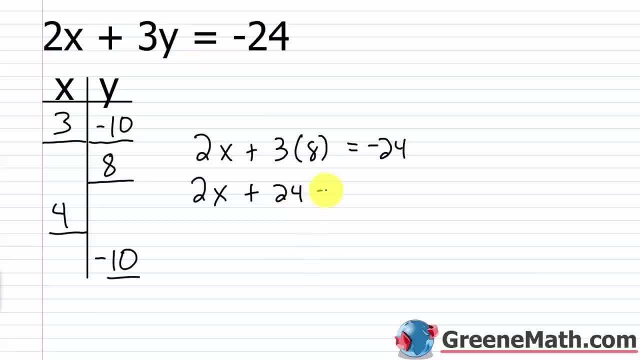 So we have 2x plus 3 times 8 is 24 equals negative 24. 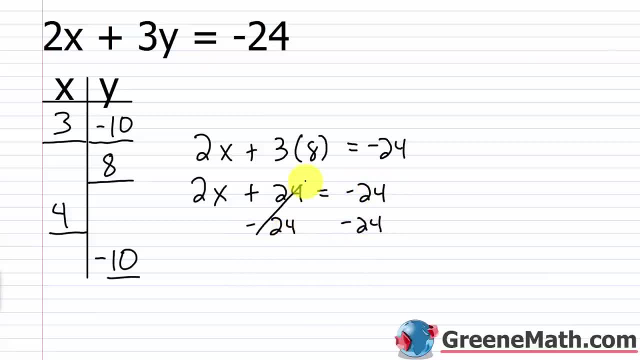 Subtract 24 away from each side. That's going to cancel. 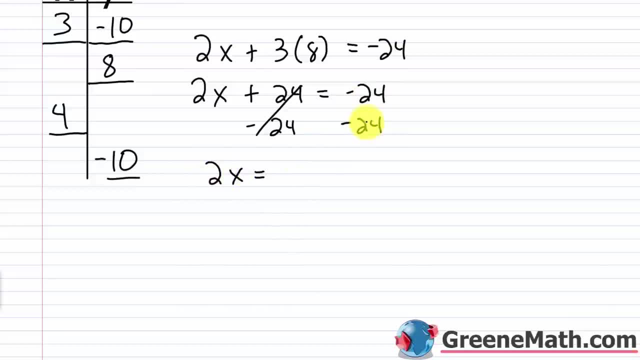 And I'm going to have 2x is equal to negative 24 minus 24 is negative 48. 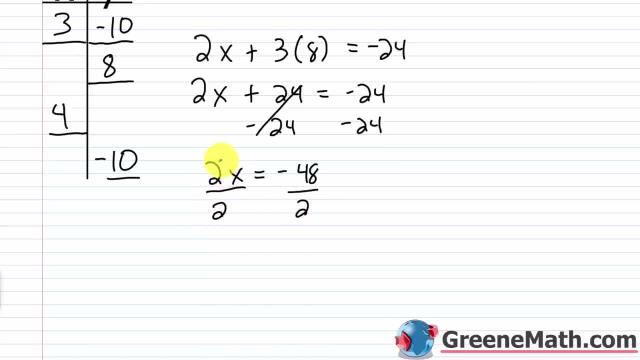 So now I can divide both sides of the equation by 2. In order to isolate x, this will cancel with this. And I'd have x is equal to negative 48 divided by 2 is negative 24. 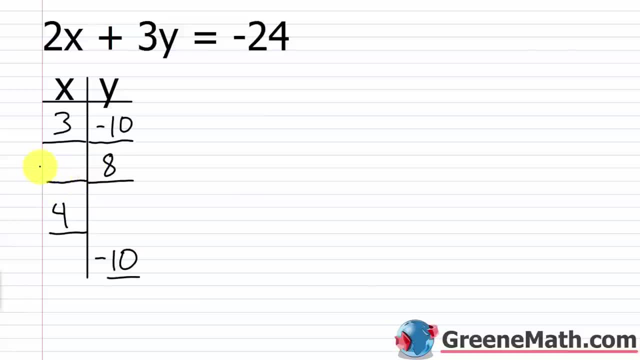 So we can come back up here and say that the missing value here is negative 24. 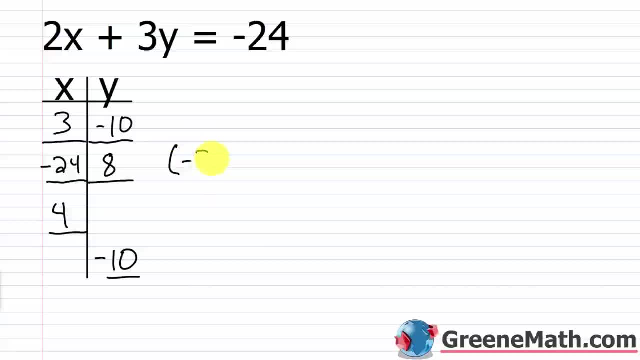 Alright, this would be another ordered pair solution. Negative 24 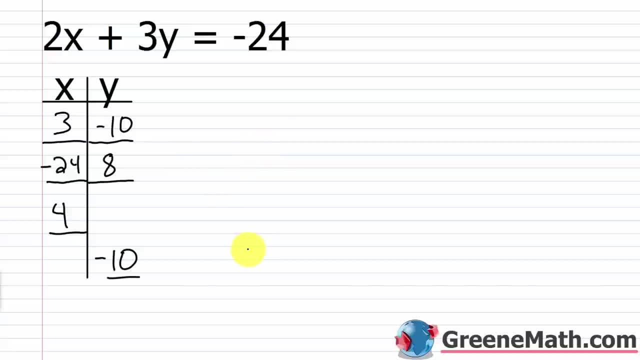 for the x value, 8 for the y value. Alright, for the next one 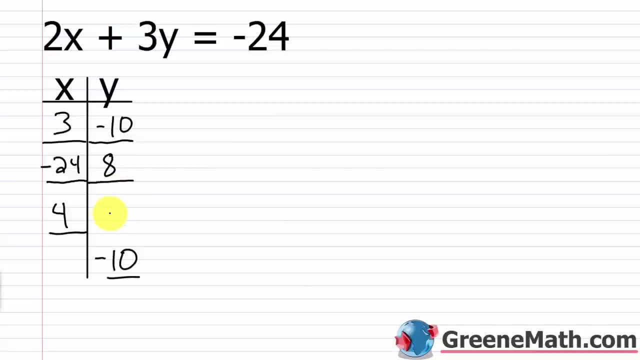 I have an x value of 4 and I want to find the unknown y value. So I'll have 2 times I have x, I'm plugging in a 4 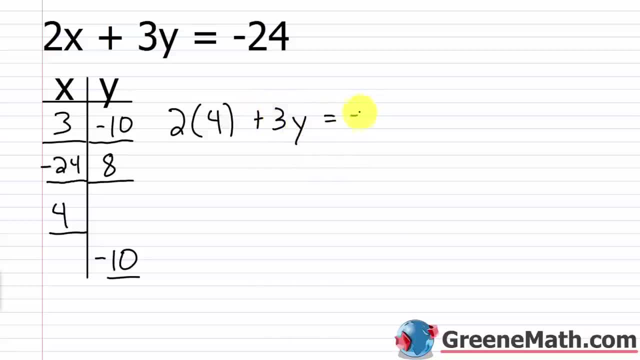 for x, plus 3y equals negative 24. So 2 times 4 is 8. So we have 8 plus 3y equals negative 24. We subtract 8 away from each side. We'll have 3y is equal to negative 32. Divide both sides of the equation by 3 so that I can 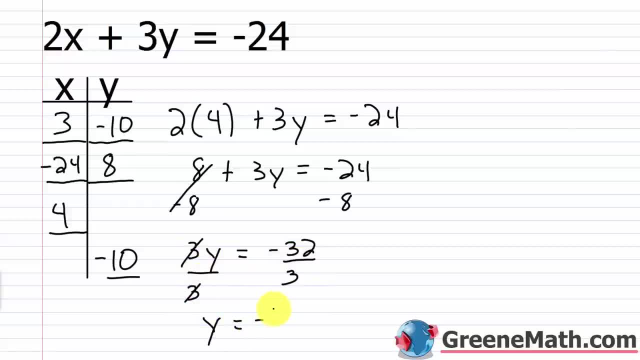 And I'll have y is equal to negative 32 thirds. 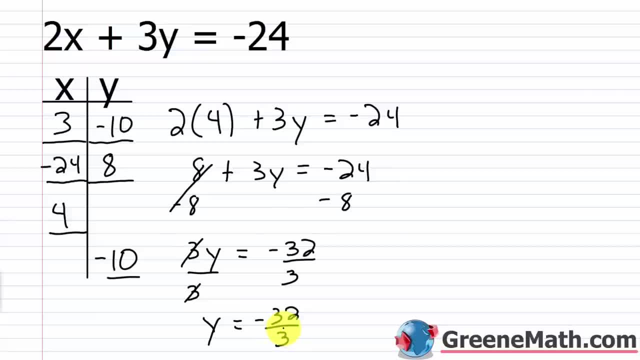 And there's nothing I can do to simplify that. If I think about 32, that's 2 to the 5th power. I can't cancel any of those factors of 2 with this 3 here. So this 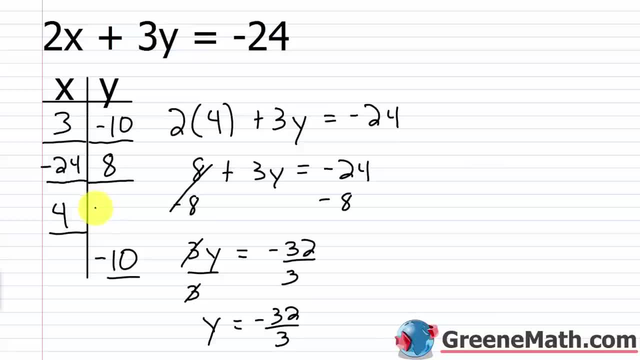 is simplified. So our missing value for y would be negative 32 thirds. 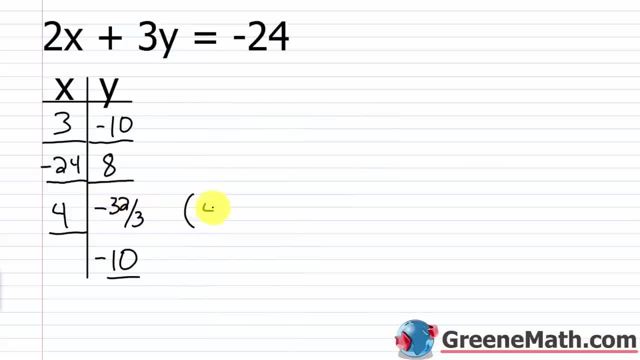 Alright, so my ordered pair solution there would be 4 comma negative 32 thirds. 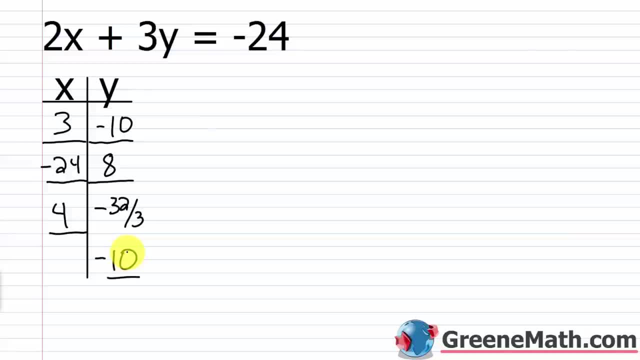 Alright, for the last one we're going to look at, we're given a y value of negative 10. So we have 2x plus 3 times I'm plugging in a negative 10 for y is equal to negative 24. 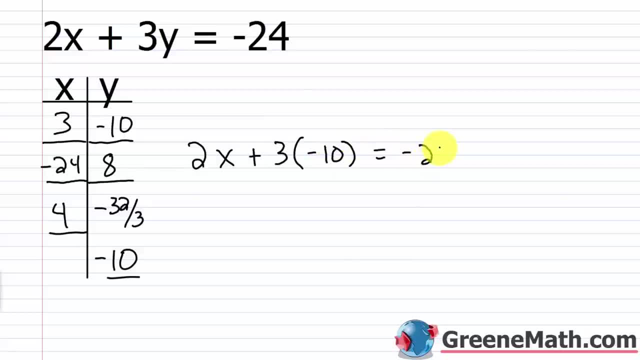 is equal to negative 24, so we then would have 2x 3 times negative. 10 is negative 30, so minus 30 equals negative 24. i'm going to add 30 to both sides of the equation. that's going to cancel. i'll have: 2x is equal to negative 24 plus 30 is going to be 6 and that can. 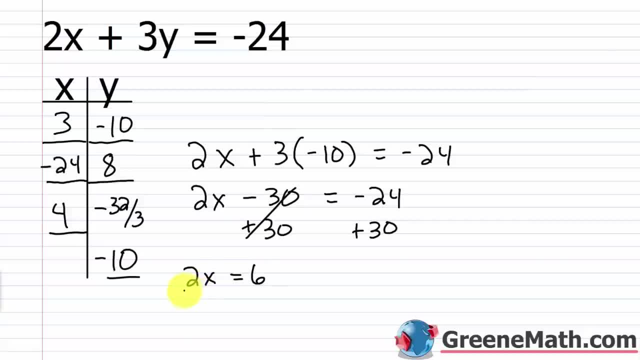 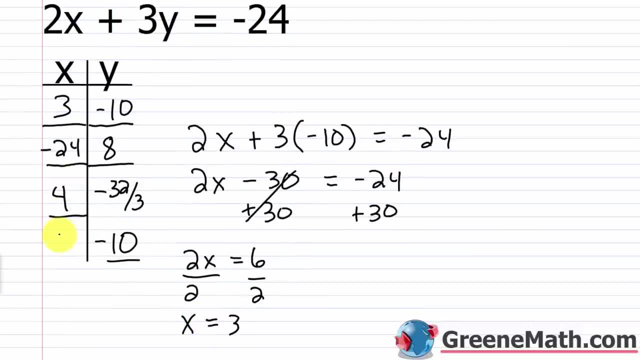 divide both sides of the equation by 2 to isolate that variable x. so divide by 2, divide by 2 and i'm going to get that x is equal to 3. all right, so i'm going to write that x is 3. it's our unknown value. 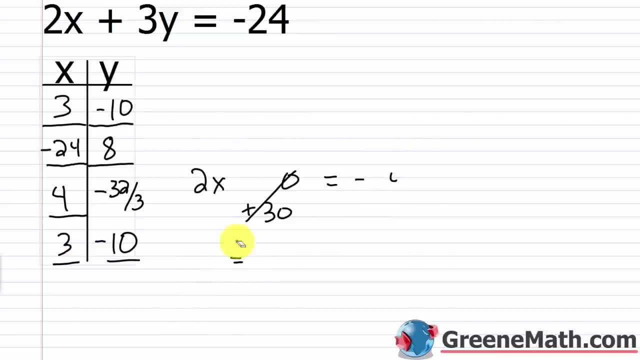 and again i'll write this as an ordered pair, just so you get a little practice doing it and seeing it. so the ordered pair would be 3 for the x value, comma negative 10 for the y value. and again you can pick any value you want for x and solve for y. or you could pick any value you want for y. 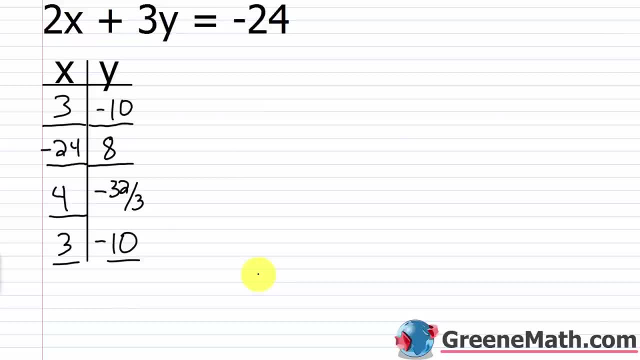 and solve for x. so, for example, let's say that i wanted to pick- i don't know- a value of 0 for x. i could say: what is the resulting y value that makes the equation true when x is 0? so i just plug in a 0 for x. so i'd have 2 times 0 plus 3y equals negative 24. 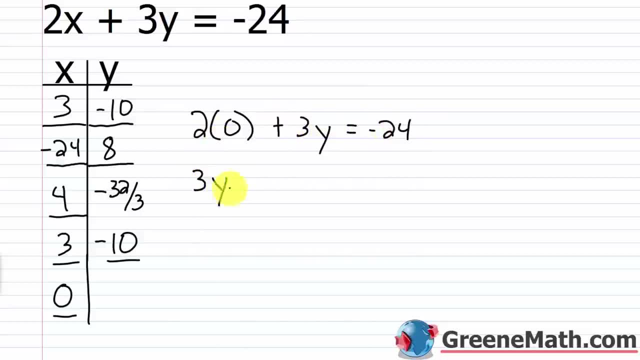 so 2 times 0 is 0. so i just have 3y equals negative 24, and this is just a linear equation of one variable. we know how to solve this already. we're just trying to isolate y at this point. so i divide both sides of the equation by 3 and i get y equals negative 8, right? so if x is 0, y is negative. 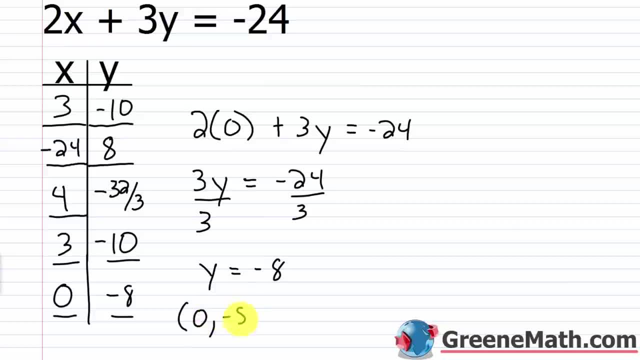 4. right, this is the ordered pair, 0 comma, negative 8, and it's a solution to this equation: 2x plus 3y equals negative 24. and again, if you want to go back and prove that to yourself, plug both of them in at the same time. so plug in a 0 for x 2 times 0 plus 3 times. plug in a negative 8 for y, so 3 times. 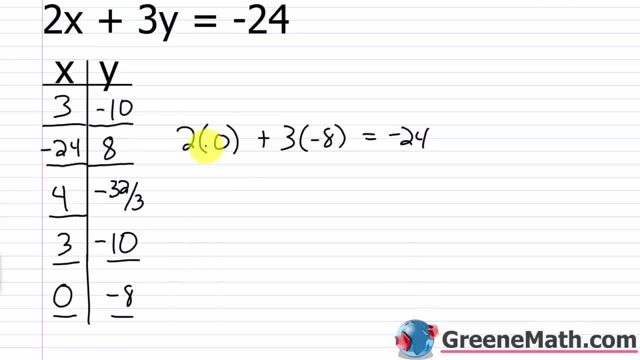 negative 8 equals negative 24.. 2 times 0 is 0, so this is gone. so we just have 3 times negative 8, that's negative 24, and that does equal negative 24.. You can see that this ordered pair, again 0 comma, negative 8, is a solution for this. 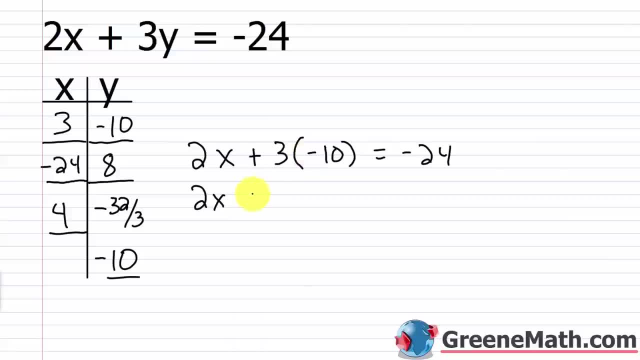 So then we'd have 2x 3 times negative 10 is negative 30 so minus 30 equals negative 24. 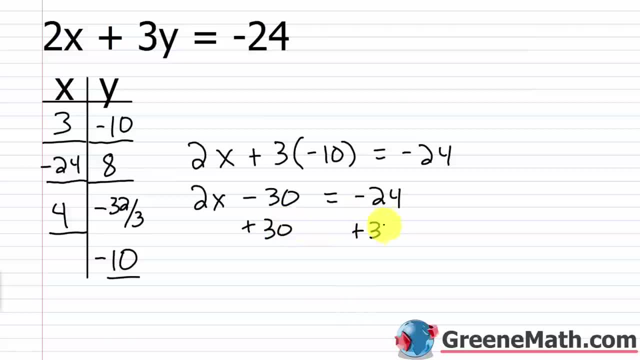 I'm going to add 30 to both sides of the equation. 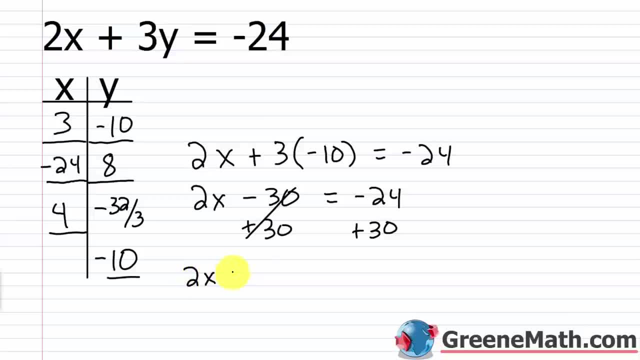 That's going to cancel. I'll have 2x is equal 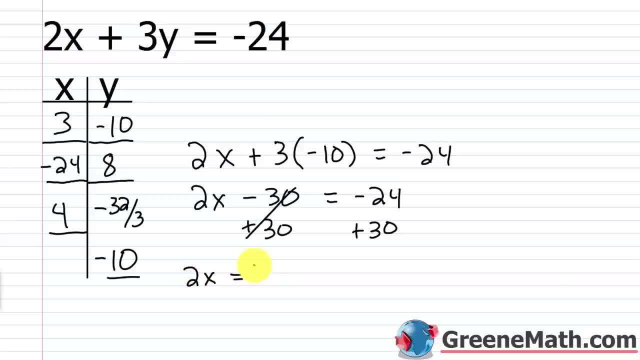 to negative 24 plus 30 is going to be 6. 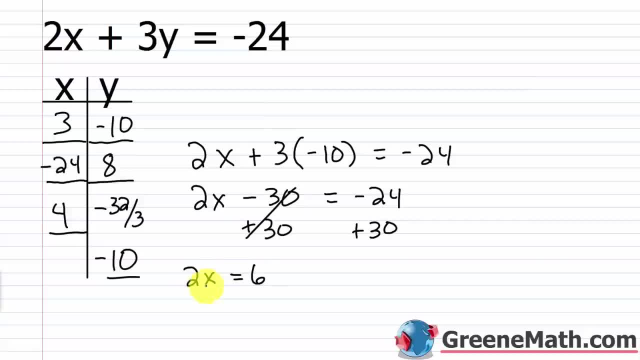 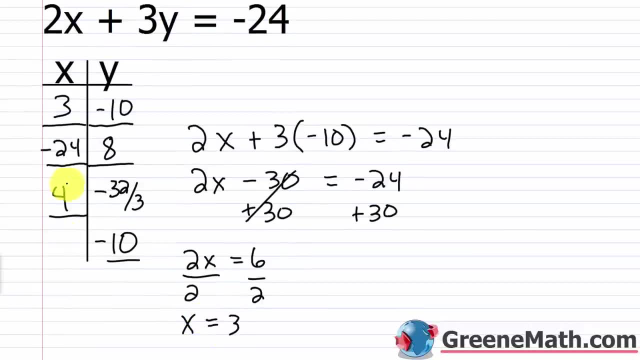 And that can divide both sides of the equation by 2 to isolate that variable x. So divide by 2, divide by 2, and I'm going to get that x is equal to 3. Alright, so I'm going to write that x is 3. That's our unknown 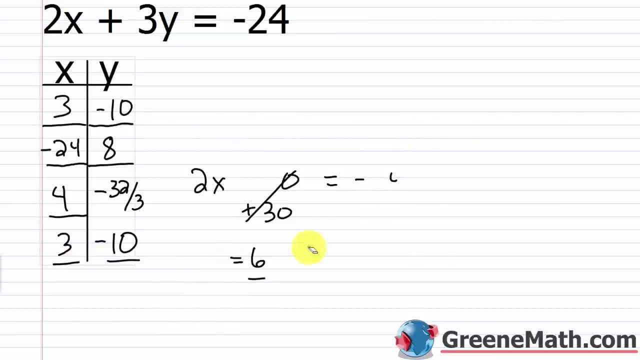 value. And again, I'll write this as an ordered pair. Just so you get a little practice doing it and seeing it. 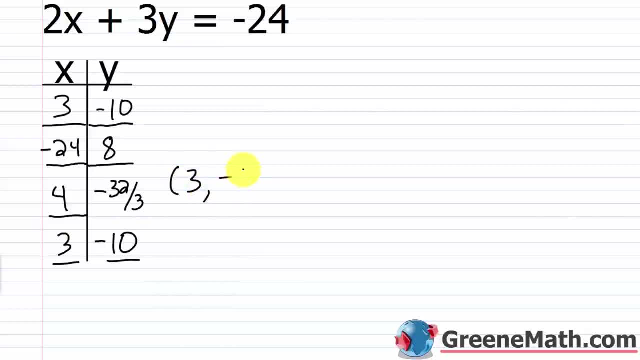 So the ordered pair would be 3 for the x value comma negative 10 for the y value. And again, 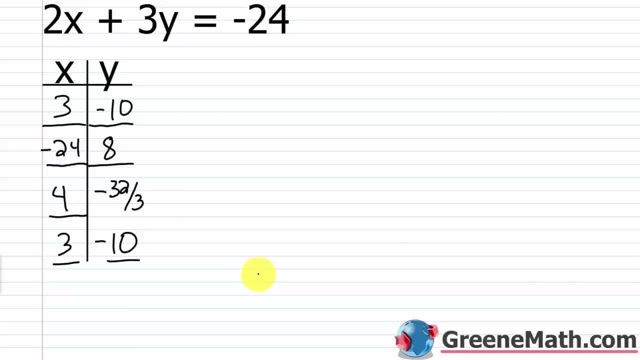 you can pick any value you want for x and solve for y. Or you could pick any value you want for y and solve for x. So for example, 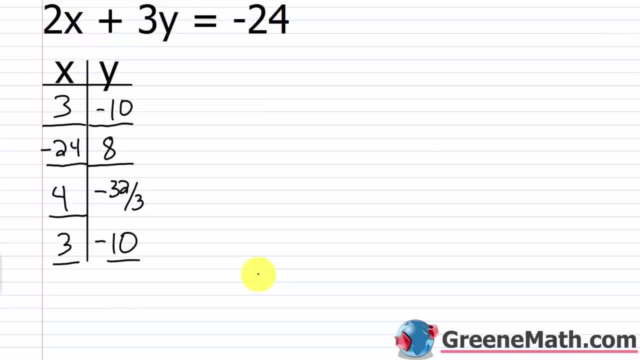 let's say that I wanted to pick I don't know, a value of 0 for x. 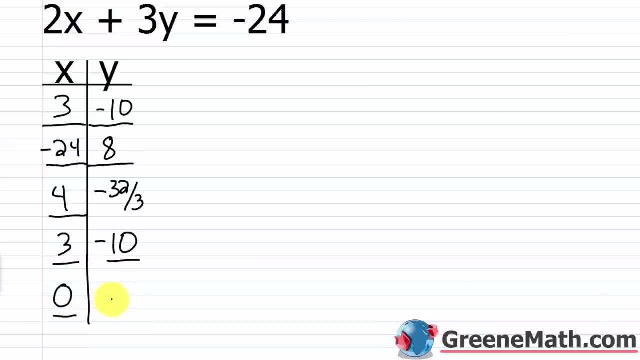 I could say, what is the resulting y value that makes the equation true when x is 0? So I just plug in a 0 for x. So I'd have 2 times 0 plus 3y equals negative 24. So 2 times 0 is 0. So I just have 3y equals negative 24. 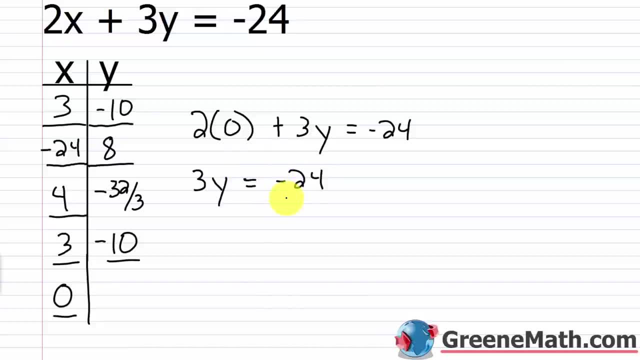 And this is just a linear equation in one variable. We know how to solve this already. We're just trying to isolate y at this point. So I divide both sides of the equation by 3. And I get y equals negative 8. So if x is 0, y is negative 8. This is the ordered pair 0 comma negative 8. 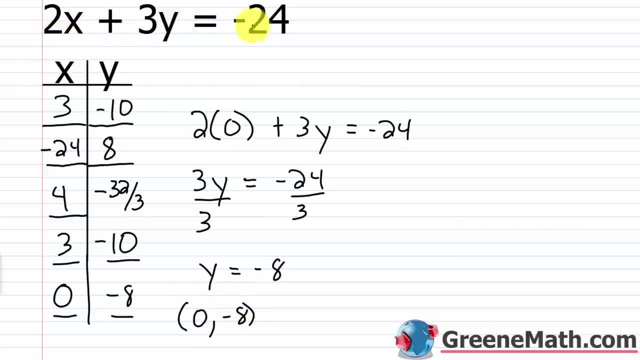 And it's a solution to this equation. 2x plus 3y equals negative 24. And again, if you want to go back and prove that to yourself, plug both of them in at the same time. So plug in a 0 for x. 2 times 0. Plus 3 times plug in a negative 8 for y. So 3 times negative 8 equals negative 24. 2 times 0 is 0. So this is gone. So we just have 3 times negative 8. That's negative 24. 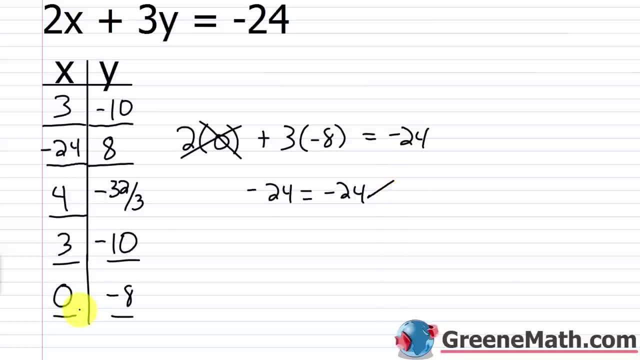 And that does equal negative 24. You can see that this ordered pair, again 0 comma negative 8, is a solution for this equation. Hello and welcome to algebra 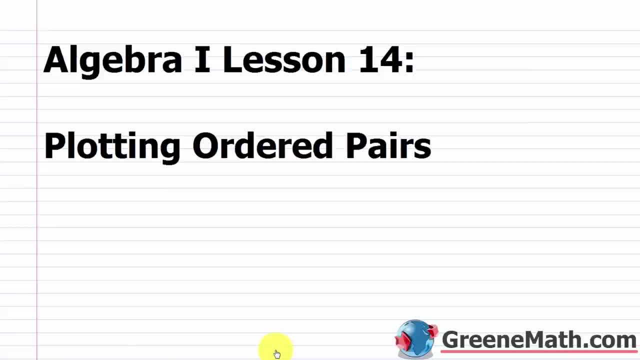 In this video we're going to learn about plotting ordered pairs. Alright so in the last lesson we learned that a linear equation in two variables has an infinite number of solutions. 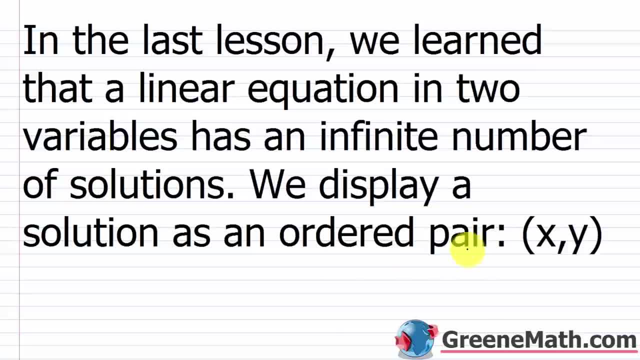 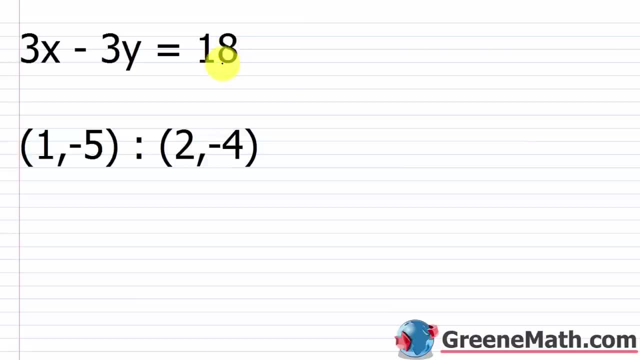 Now we display a solution as an ordered pair. So you have an x value comma a y value. And it's always in that order. The x value is on the left. The y value is on the right. So for example, in this equation we have 3x minus 3y equals 18. And we have 2 ordered pairs here that are proposed solutions. 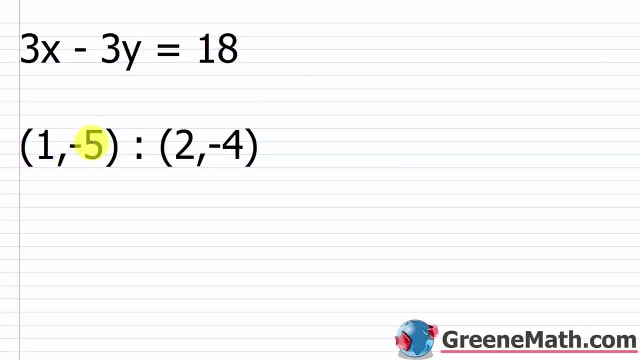 So if this ordered pair, 1 comma negative 5 is a solution to this equation, that means that I can take this value here and plug it in for x. This value here and plug it in for y. And I should get a true statement. The left and the right side should be equal. So let's see if it is. 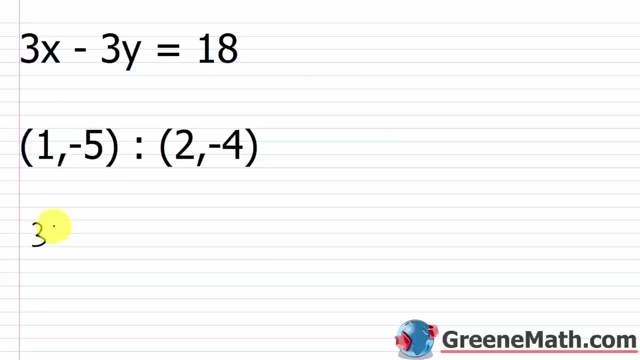 So I would take a 1 and plug it in for x. So 3 times 1 minus. I take a negative 5 and plug it in for y. So I'd have 3 times negative 5. And this should be equal to 18. 3 times 1 is 3. Negative 3 times negative 5 is positive 15. So plus 15. 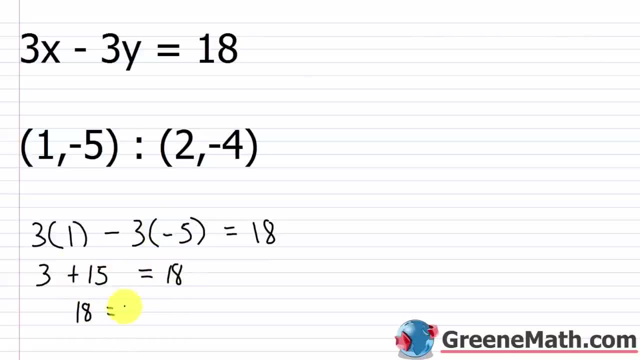 This should equal 18. And it does. 18 equals 18. So that works out. 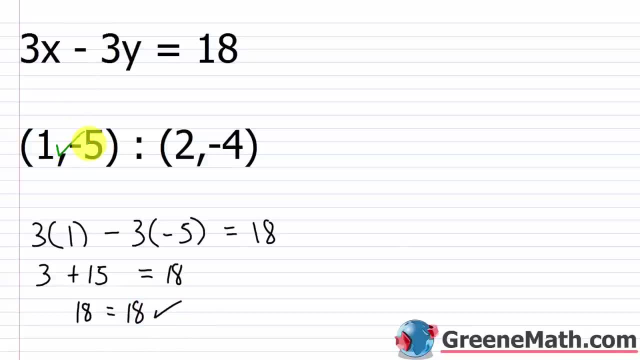 So we can say that this ordered pair 1 comma negative 5 is a solution for this equation. 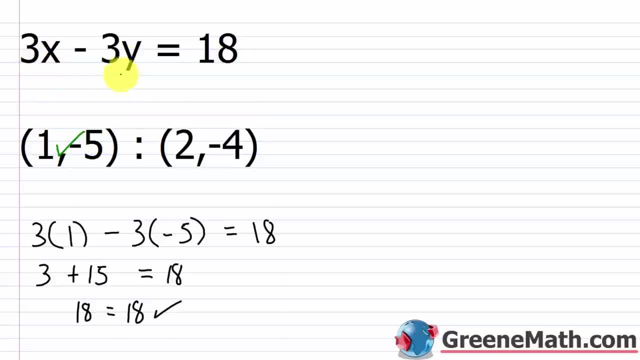 Again, because when I plug in a 1 or x and a negative 5 for y, I get a true statement. 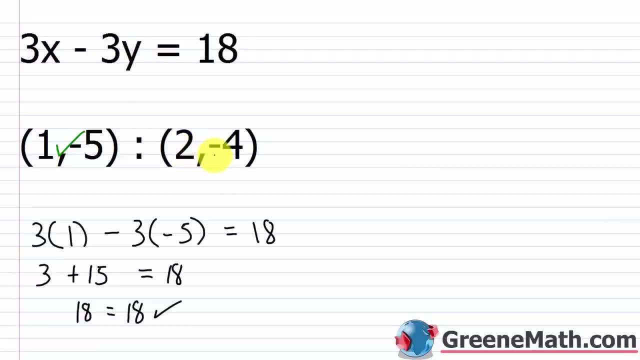 Let's do the same thing with this ordered pair 2 comma negative 4. Alright, so we'd have 3 times x. Our value for x is 2. Minus 3 times y. Our value for y is negative 4. And this equals 18. So 3 times 2 is 6. 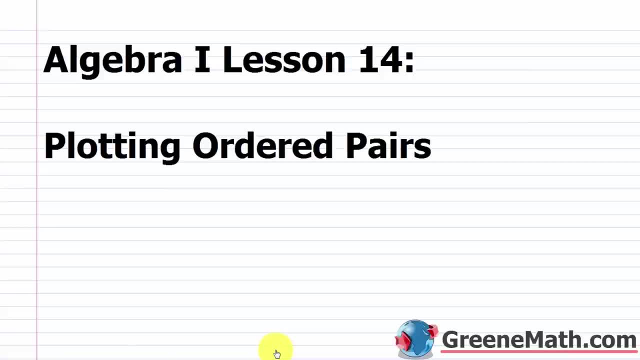 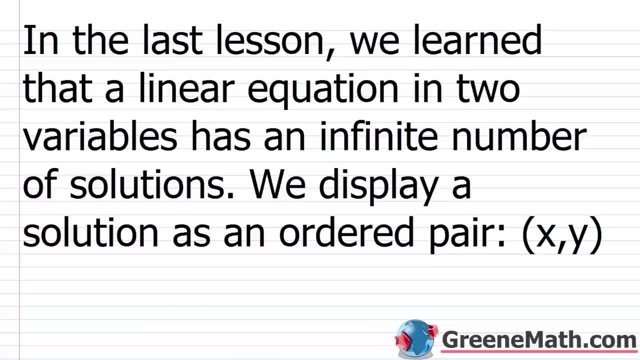 equation. Hello and welcome to Algebra 1, lesson 14.. In this video we're going to learn about plotting ordered pairs. Alright, so in the last lesson we learned that a linear equation in two variables has an infinite number of solutions. Now we display a solution as an ordered pair, so you have an x value comma, a y value. 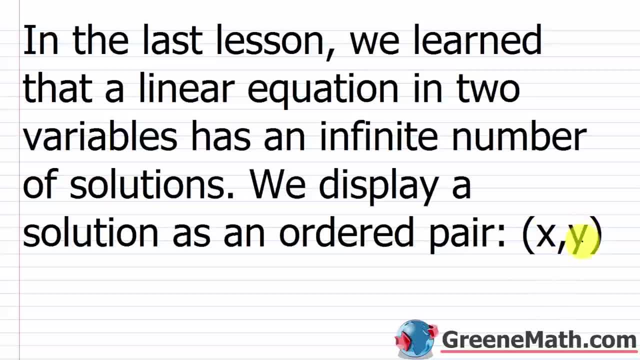 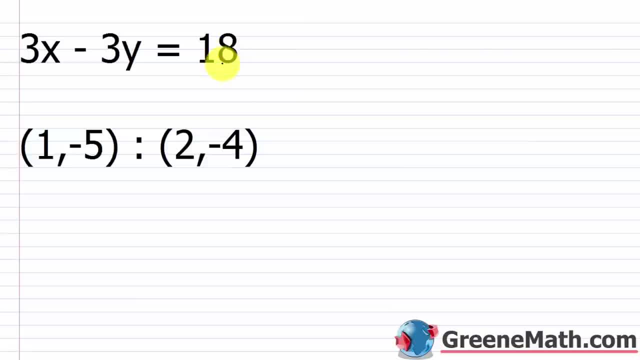 and it's always in that order: the x values on the left, the y values on the right. So for example, in this equation we have 3x minus 3y equals 18 and we have two ordered pairs here that are proposed solutions. So if this ordered pair 1 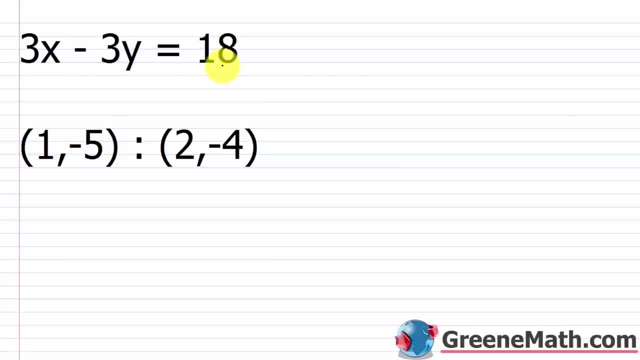 comma negative 8 is a solution for this equation, then we have: 3x minus 3y equals 18 and we have two ordered pairs here that are proposed solutions. So if this ordered pair, 1 comma negative 5, is a solution to this equation, that means that I can take this: 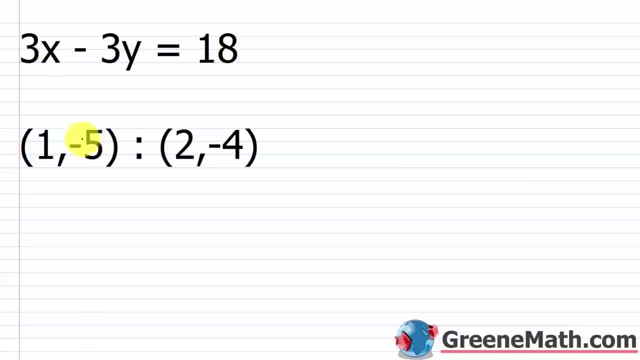 value here and plug it in for x, this value here and plug it in for y, and I should get a true statement right. the left and the right side should be equal. So let's see if it is So. I would take a 1 and plug it in for x, so 3 times 1 minus. 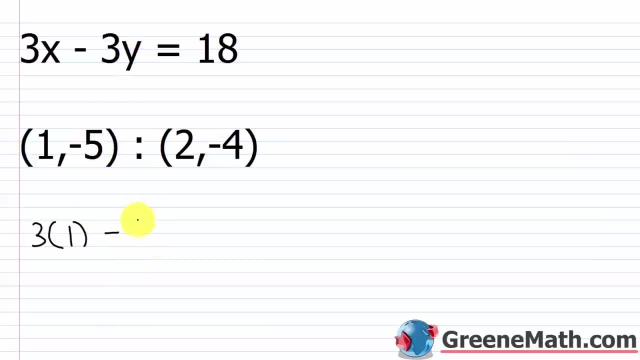 I take a negative 5 and plug it in for y, so I'd have 3 times negative 5 and this should be equal to 18.. 3 times 1 is 3 negative. 3 times negative 5 is positive 15. so plus 15 it should. 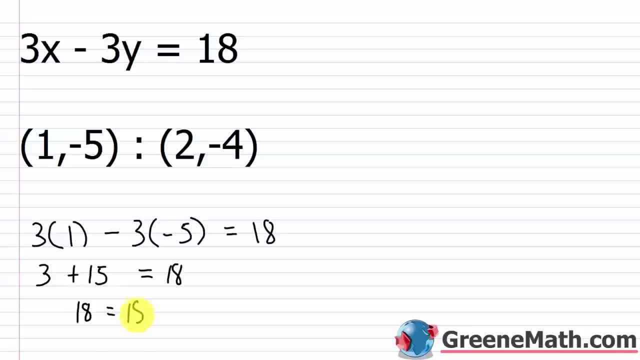 equal 18 and it does 18 equals 18.. So that works out. So we can say that this ordered pair, 1 comma negative 5, is a solution for this equation again, because when I plug in a 1 for x and a negative 5 for y, I get a true statement. Let's do. 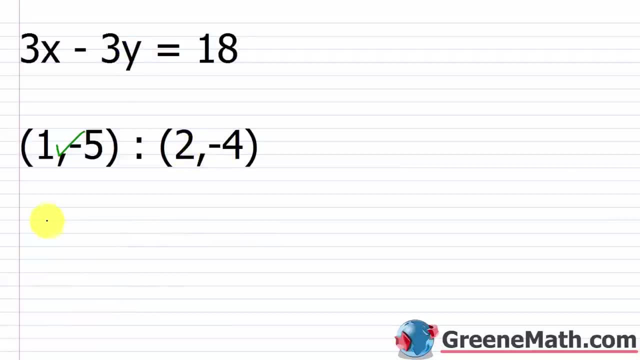 the same thing with this ordered pair. 2 comma, negative 4.. Alright, so we'd have 4.. So we'd have 3 times x. our value for x is 2, minus 3 times y: our value for y is negative. 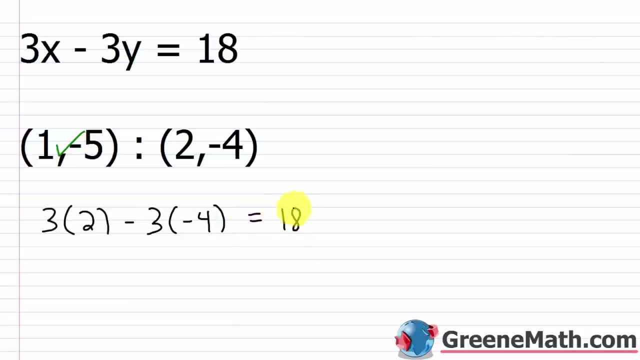 4, and this equals 18.. So 3 times 2 is 6, then we have negative, 3 times negative 4, that's 12, so plus 12 equals 18, and it does 6 plus 12 is 18, so you get 18 equals 18.. 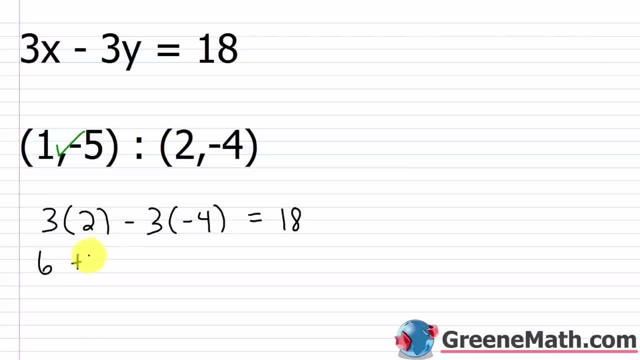 Then we have negative 3 times negative 4. That's 12. So plus 12 equals 18. And it does. 6 plus 12 is 18. So you get 18 equals 18. And so we can say that this ordered pair 2 comma negative 4 is also a solution for this equation 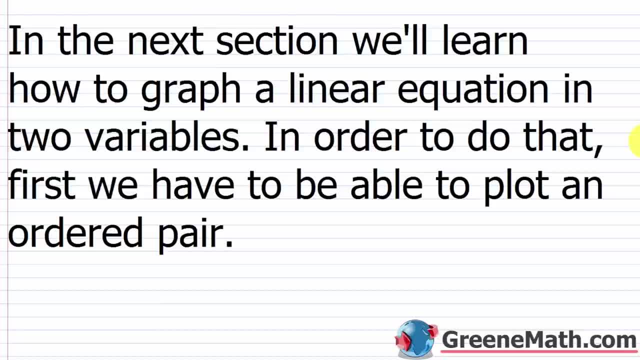 3x minus 3y equals 18. So you might be asking yourself, what are we going to do with these ordered pairs? Well, in the next section we're going to learn how to graph a linear equation in two 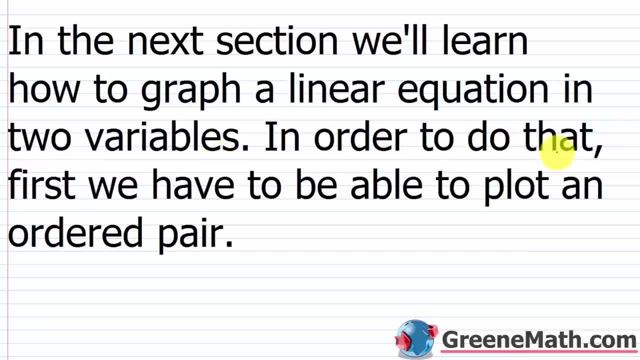 variables. But in order to do that, we first have to be able to plot an ordered pair. Alright, so in order to talk about plotting ordered pairs, 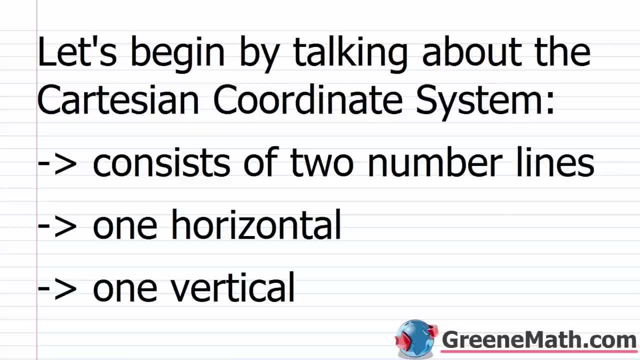 we're going to first begin by talking about something known as the Cartesian coordinate system. The, again, Cartesian coordinate system. Now, this might be a source of some confusion for you because this has many names. And probably in your textbook it'll be called Cartesian coordinate system and then after that they start calling it the rectangular 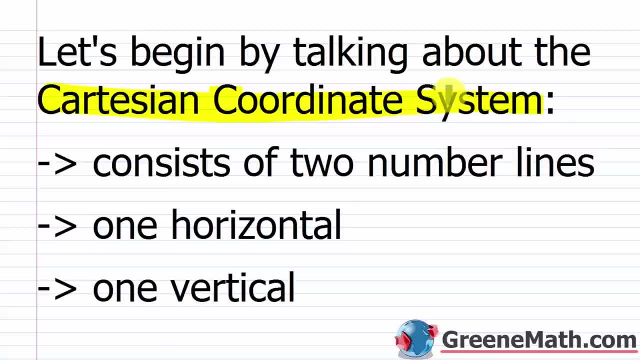 coordinate system and sometimes they just call it the coordinate plane. And a lot of students will be like, well, what is this now? They're all the same thing. 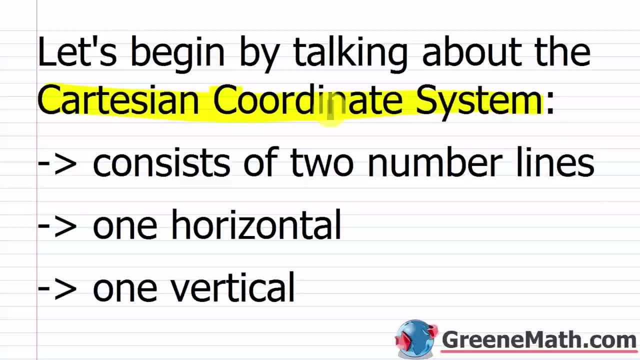 It's named after its inventor and you'll probably read the story as a side note in your textbook where it says, you know, he's lying in bed and he's watching a fly move and he comes up with this coordinate plane. And so, long story short, it's named after him and it's called the Cartesian coordinate system but you might hear it called something else. Most of the time I'm just going to call it a coordinate plane because it's nice and simple. 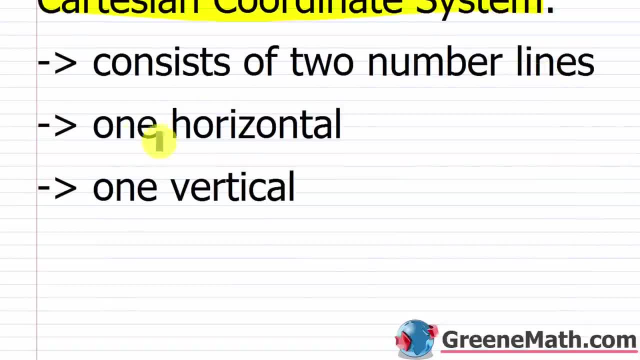 What you need to know is that it consists of two number lines. One's horizontal and one's vertical. 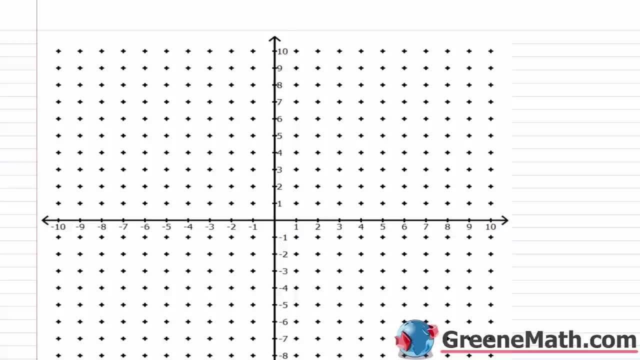 So let's take a look at this thing. Alright, so 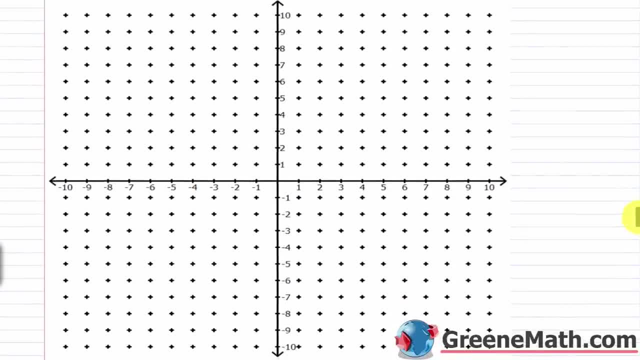 here's an example of the coordinate plane. Now if you just look at this right here, starting here and going to the right, this is the number line we've been 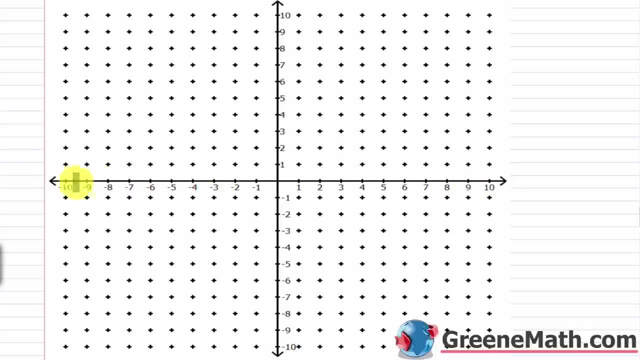 working with for a long time now. It's a horizontal number line and you'll notice that if I were to tell you this is the point zero, 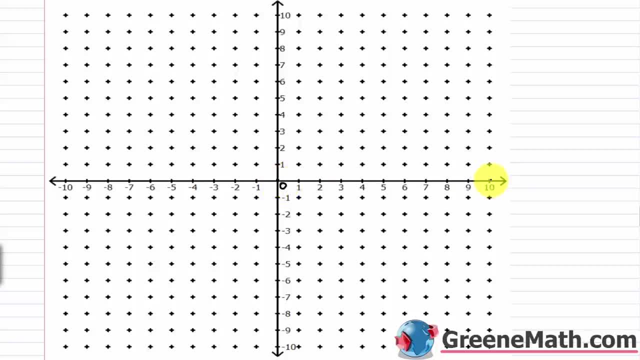 everything to the right of zero is a positive number. We know that already. 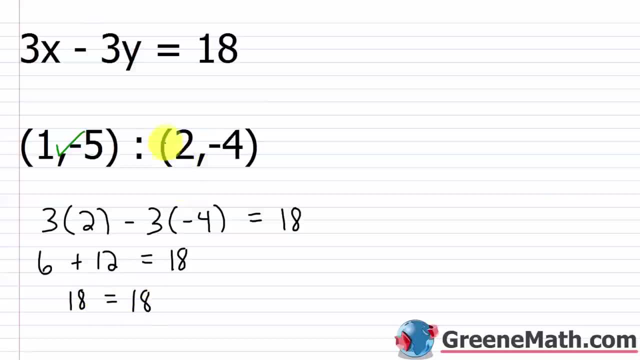 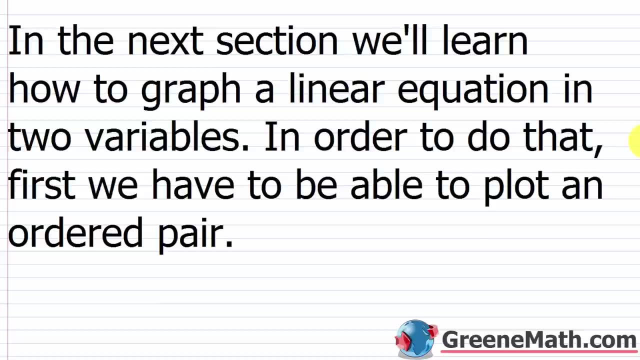 And so we could say that this ordered pair- 2 comma negative 4, is also a solution for this equation: 3x minus 3y equals 18.. So you might be asking yourself what are we going to do with these ordered pairs? 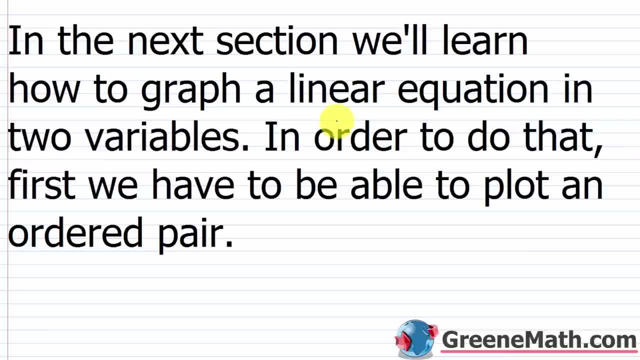 Well, in the next section we're going to learn how to graph a linear equation in two variables. But in order to do that, we first have to be able to plot an ordered pair. Alright, so in order to talk about plotting ordered pairs, we're going to first begin. 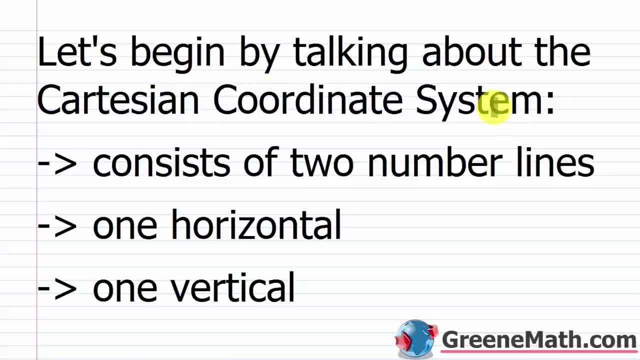 by talking about something known as the Cartesian Coordinate System, the again Cartesian Coordinate System. Now, this might be a source of some confusion for you, because this has many names And probably in your textbook it'll be called Cartesian Coordinate System and then after: 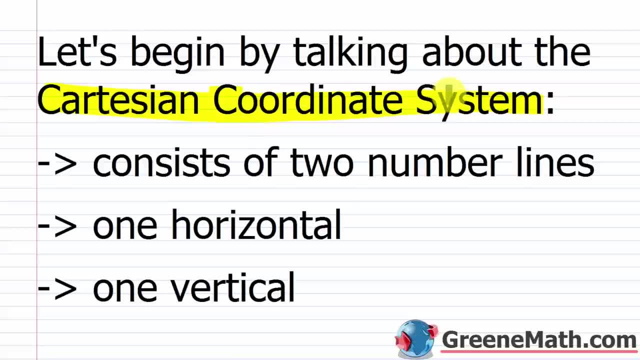 that they start calling it the Rectangular Coordinate System and sometimes they just call it the Coordinate Plane, and a lot of students will be like, well, what is this now? What is this? They're all the same thing. Okay, It's named after its inventor. 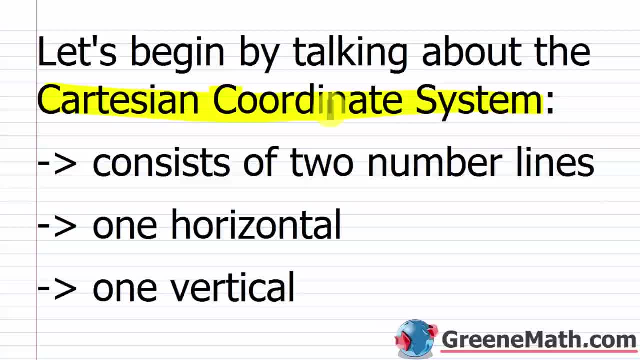 Okay, I'm going to give you a story as a side note in your textbook where it says: you know, he's lying in bed and he's watching a fly move and he comes up with this, this Coordinate Plane. And so, long story short, it's named after him and it's called the Cartesian Coordinate. 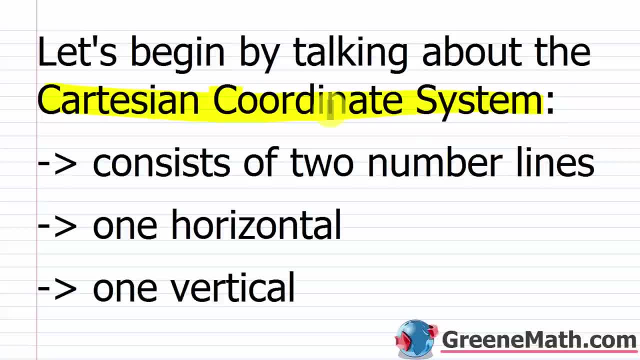 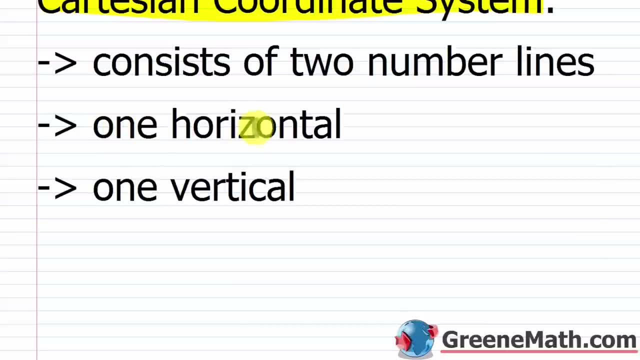 System, but you might hear it called something else Most of the time. I'm just going to call it a Coordinate Plane because it's nice and simple. What you need to know is that it consists of two number lines: One's horizontal and one's vertical. 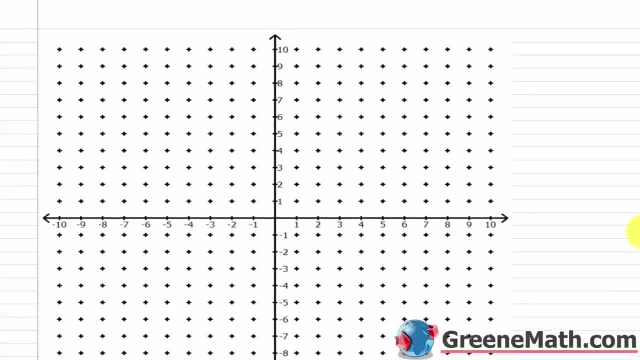 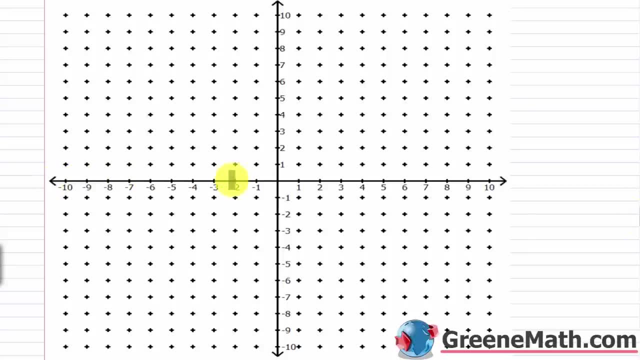 So let's take a look at this thing. Alright, so here's an example of. Okay, So here's an example of the Coordinate Plane. Now, if you just look at this right here, starting here and going to the right, this is the number. 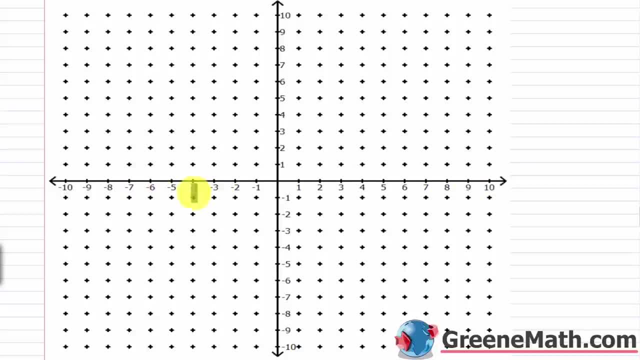 line we've been working with for a long time now. It's a horizontal number line and you'll notice that if I were to tell you this is the point- zero- everything to the right of zero, is a positive number. We know that already. 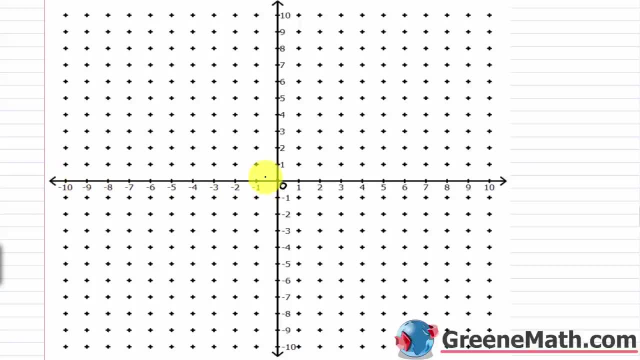 Everything to the left of zero is a negative number. We know that already. Okay, So what happens? is this vertical number line okay, this vertical number line, and the way this works is that everything above zero is positive, everything below zero is negative. 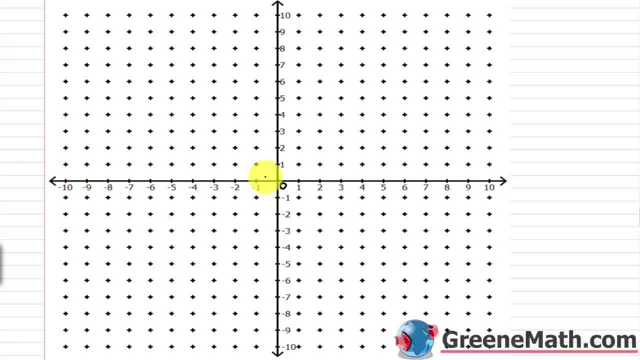 Everything to the left of zero is a negative number. We know that already. 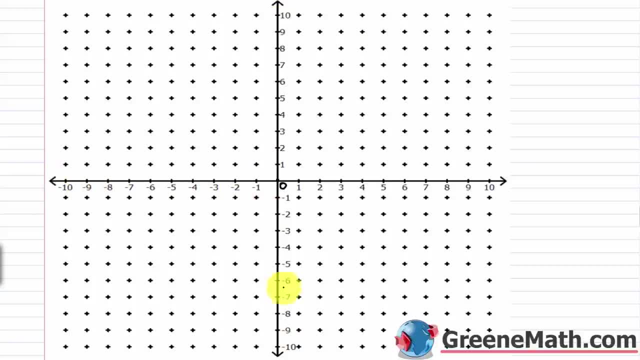 But new to us is this vertical number line. 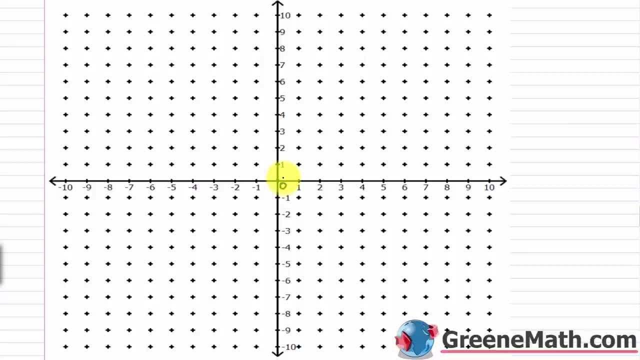 This vertical number line. And the way this works is that everything above zero is positive. Everything below zero is 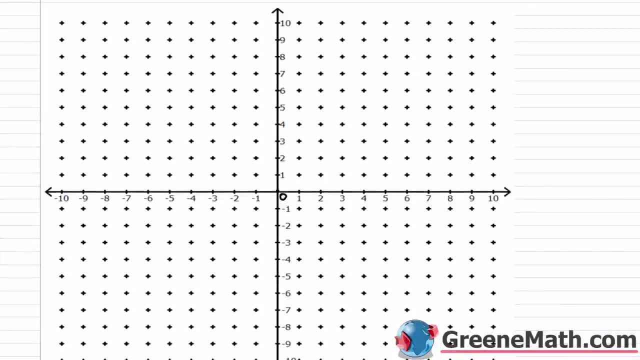 negative. So a couple of important points here. 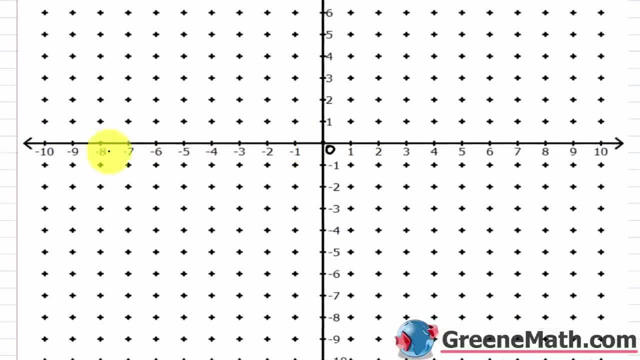 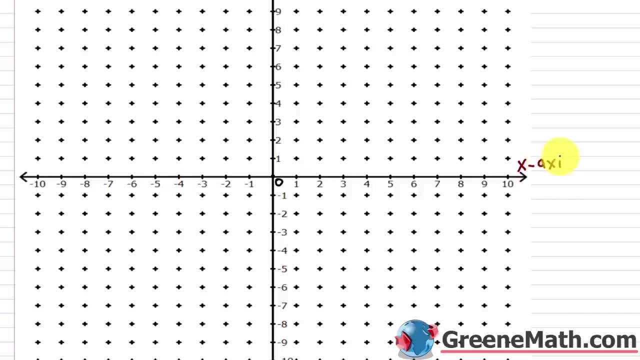 The first thing that you need to know is that the horizontal axis, this axis that's going left to right, this is the x axis. This is the x axis. And actually let me write this right here. 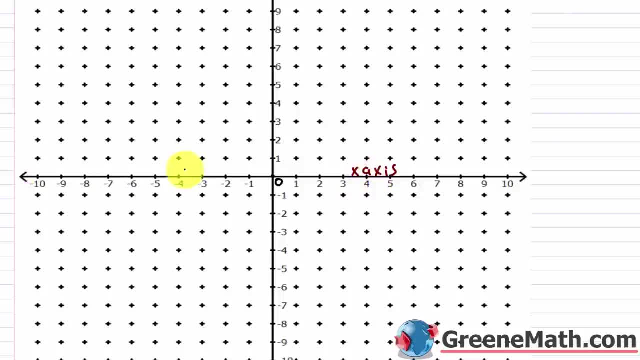 x axis. Okay, so it's going left 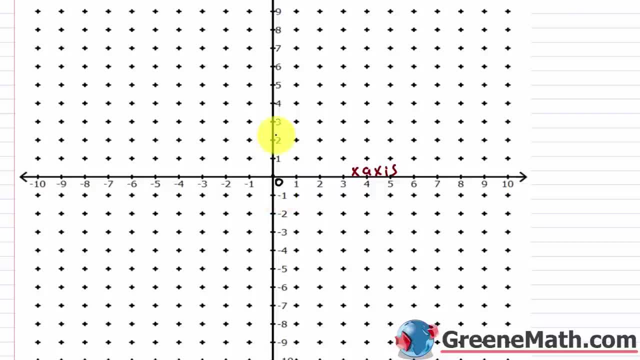 to right. Now the y axis is going up and down. 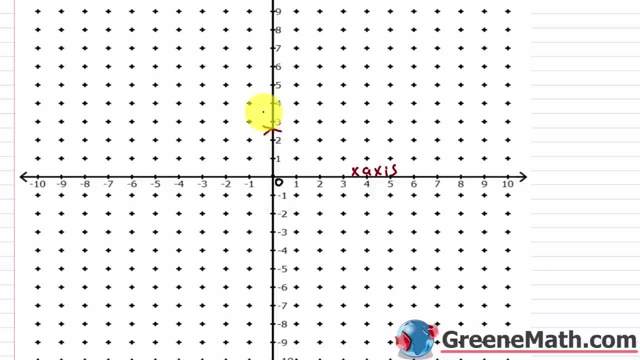 So let me kind of write this like this. This is the y axis. 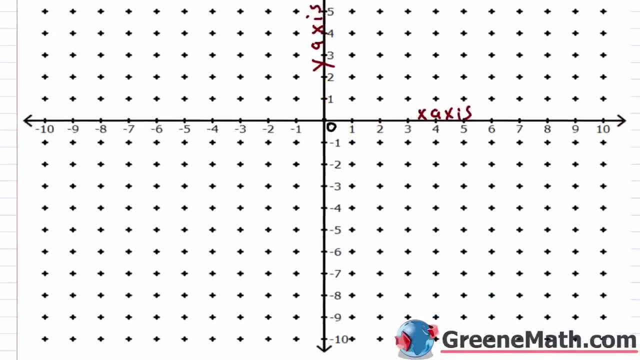 Now the place where they intersect, you'll see it right here. This comes down and meets this right here. 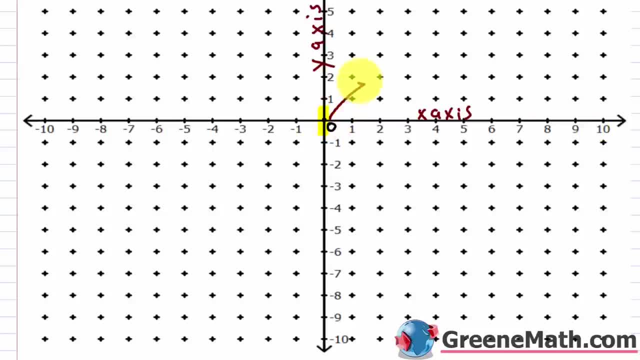 See where I have the zero there? That's called the origin. That's the place of intersection. So this is the origin. 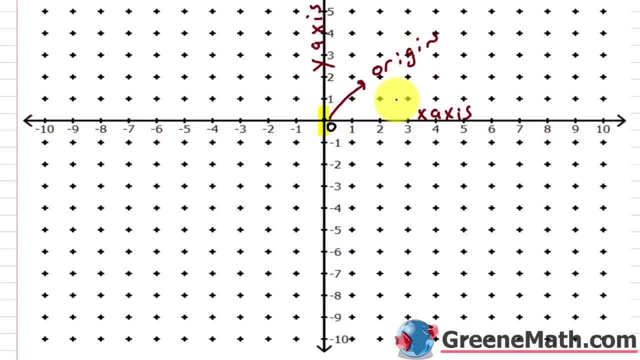 Alright, so the last little piece of information I'm going to give you about this. The coordinate plane 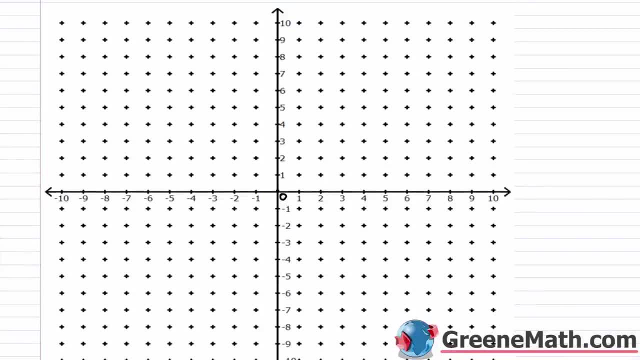 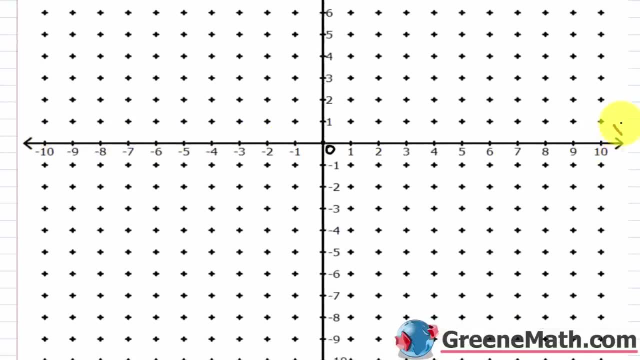 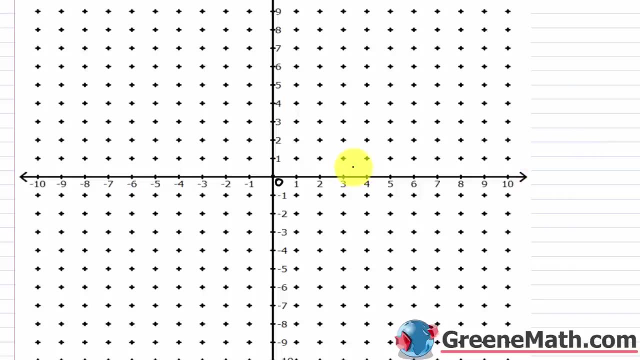 So a couple of important points here. The first thing that you need to know is that the horizontal axis, this axis that's going left to right, this is the x-axis. This is the x-axis And actually let me write this, Let me write this right here: 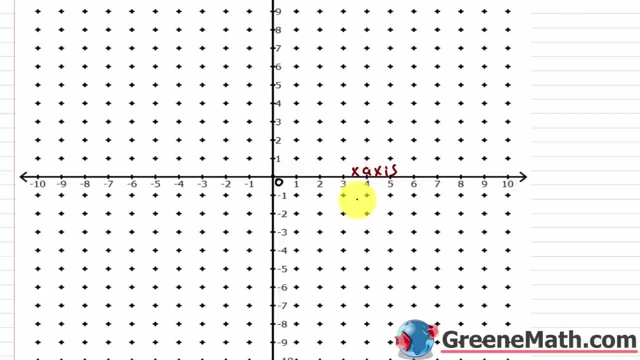 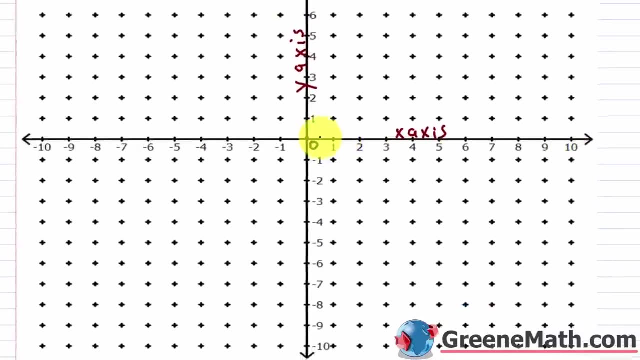 X-axis. Okay, So it's going left to right. Now the y-axis is going up and down, So let me kind of write this like this: This is the y-axis Now, the place where they intersect. you'll see it right here, right? 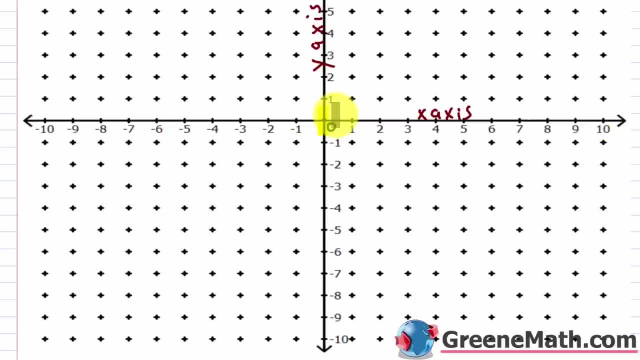 This comes down and meets this right here. See where I have the zero there. That's called the origin. That's the place of intersection. So this is the origin. All right, So the last little piece of information I'm going to give you about this: the coordinate. 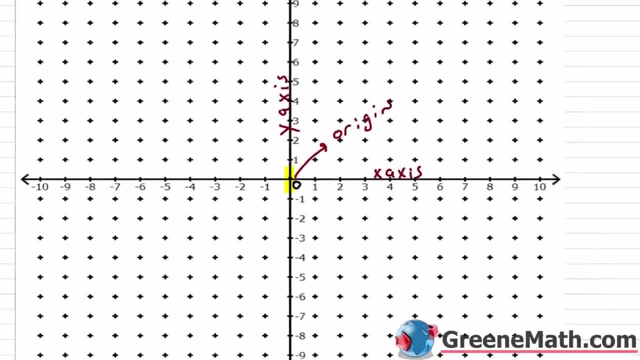 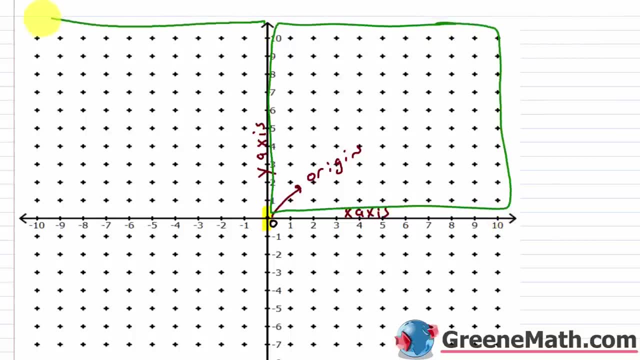 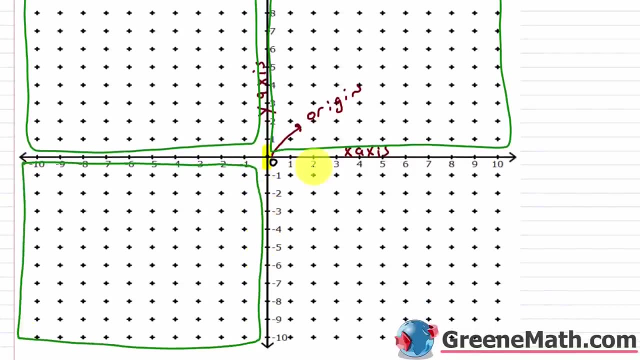 plane has what we call quadrants, So you can kind of box this off into four areas. So this is an area, this is an area, this is an area and this is an area. So this first area, all the way to the right, the top right, 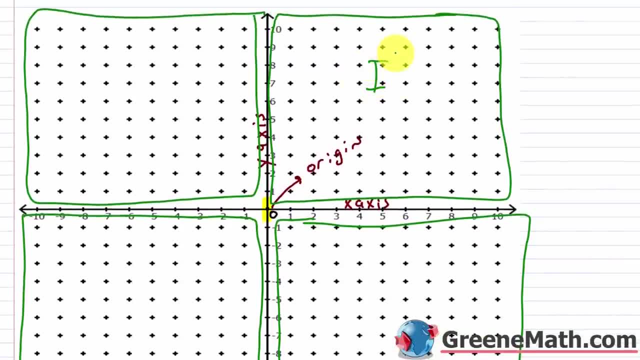 This is quadrant number one, Quadrant number one, And let me erase this so I can show you something. Let me erase all these. In quadrant one, the x values are positive. So you see that we exist in a plane of space where all the x values are to the right of 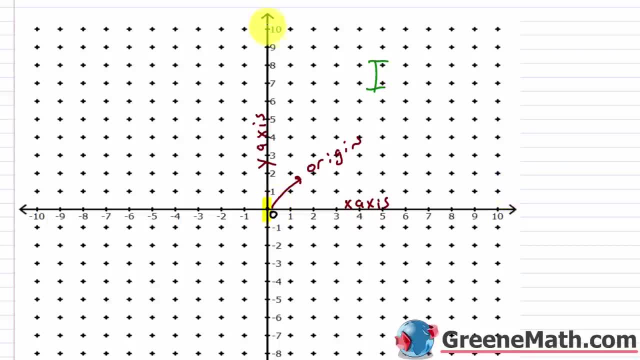 zero and all the y values are above zero. So in quadrant one, your ordered pair is going to have an x value that's positive and a y value that's positive. Okay, So your x is positive, Your y is positive. Now, that's important for you to remember because that might come up on a test. 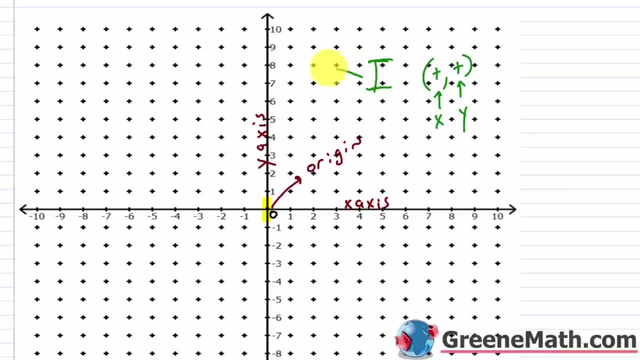 Now we move counterclockwise, So we go kind of this direction. So the next quadrant is over here. This is quadrant two, And in this quadrant you'll notice that my x values are to the left of zero, So they're going to be negative. 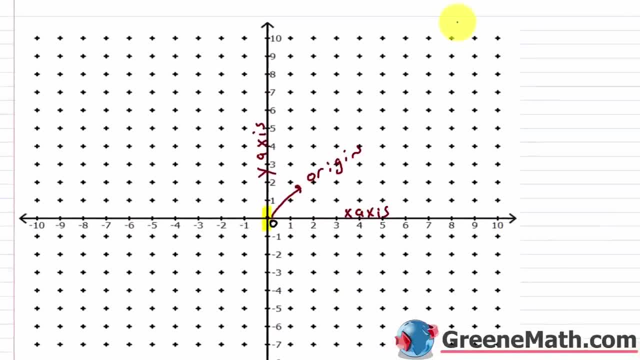 has what we call quadrants. So you can kind of box this off into four areas. 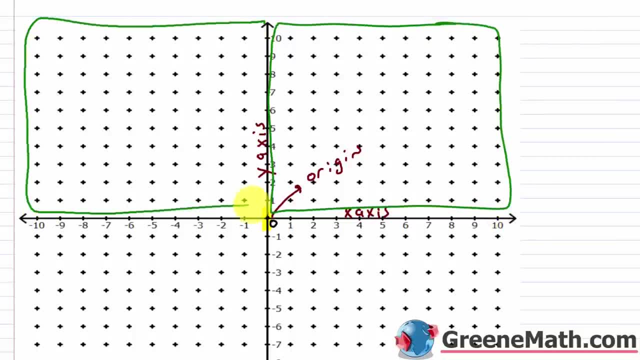 So this is an area. This is an area. This is an area. 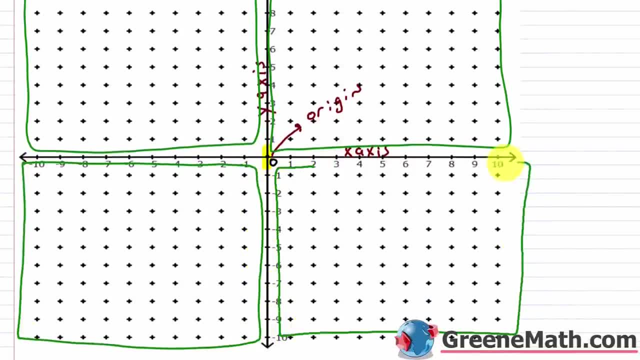 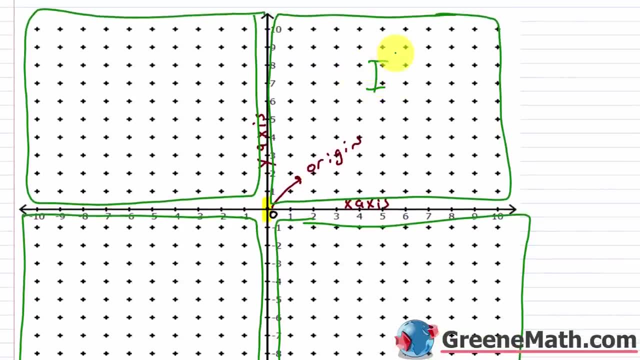 And this is an area. So this first area all the way to the right. The top right. This is quadrant number one. And let me erase this so I can show you something. Let me erase all these. 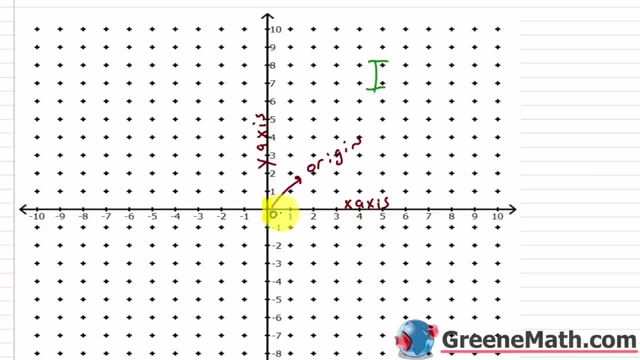 In quadrant one, the x values are positive. So you see that we exist in a plane of space where all the x values are to the right of zero. And all the y values are above zero. So in quadrant one, your ordered pair is going to have an x value that's positive. 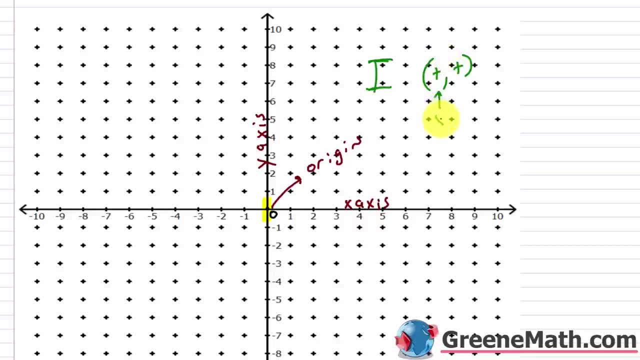 And a y value that's positive. So your x is positive. Your y is positive. Now that's important for you to remember because that might come up on a test. 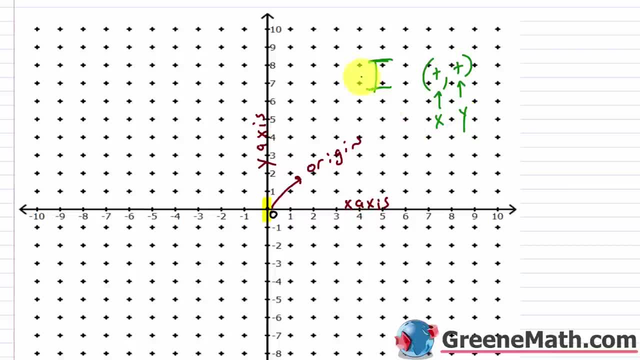 Now we move counter clockwise. So we go kind of this direction. So the next quadrant is over here. This is quadrant two. 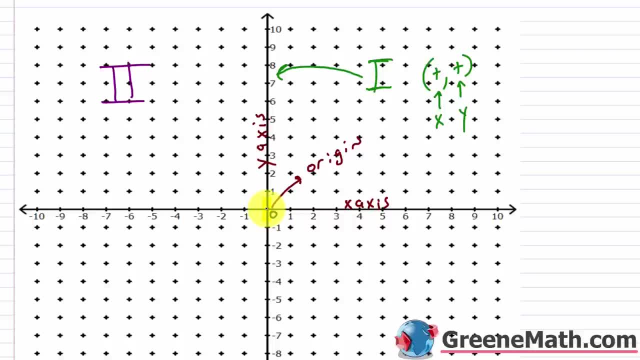 And in this quadrant, you'll notice that my x values are to the left of zero. So they're going to be negative. 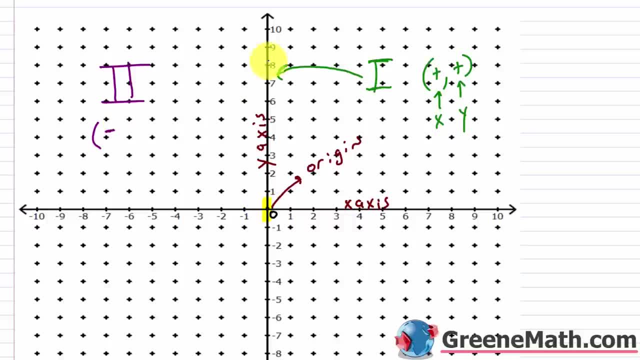 My y values are still above zero so they're going to be positive. 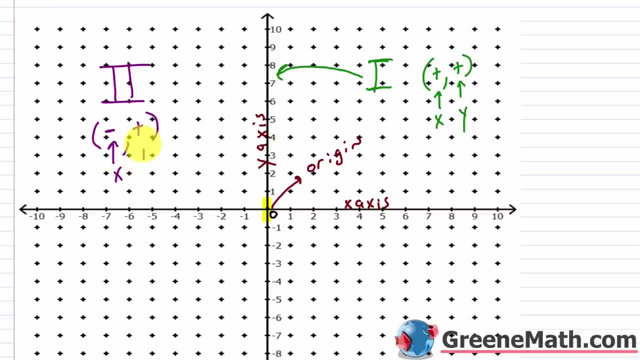 So this is my x. This is my y. So x is negative here. y is positive. 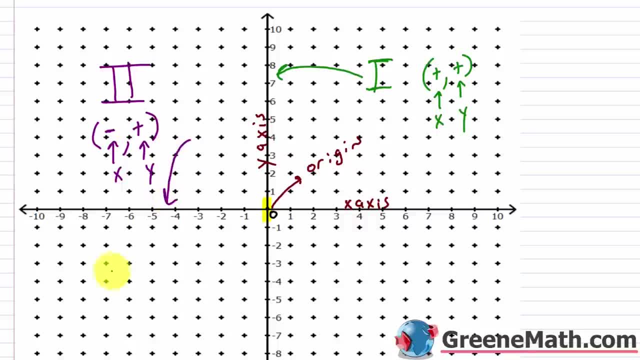 Alright, now we continue going this way. Now this is quadrant three. 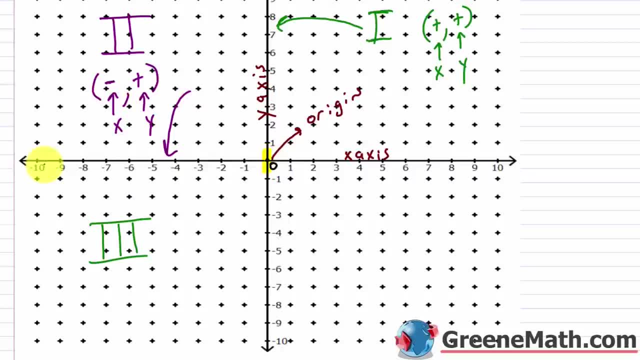 Now in this quadrant, we're to the left of zero so our x values are negative. And we're below zero so our y values are also negative. So again, this is my x values. These are Alright, then the final quadrant, we go this way. 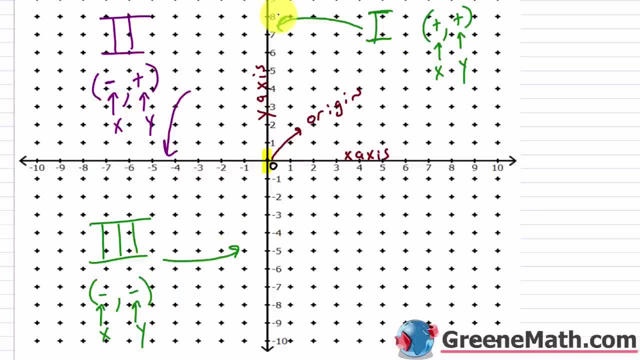 Again, it's counter clockwise so it just goes this way. 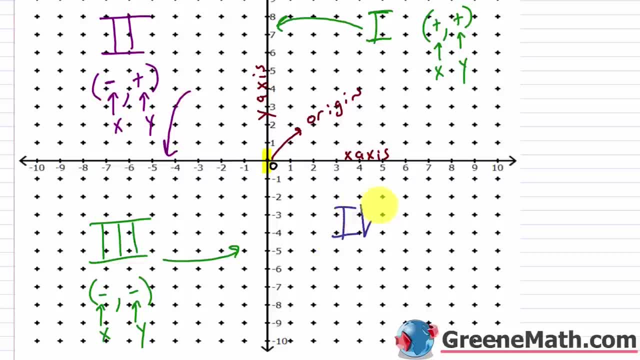 We end up here, and this is quadrant four. 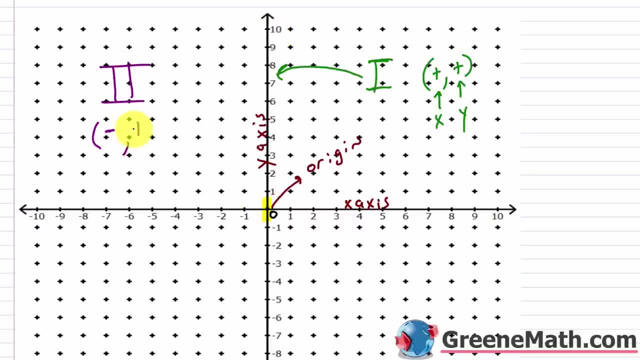 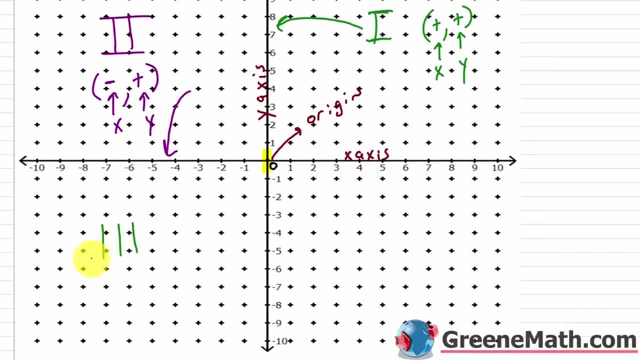 My y values are still above 0, so they're going to be positive. So this is my x, this is my y. So x is negative here, y is positive. Now we continue going this way. Now this is quadrant 3.. 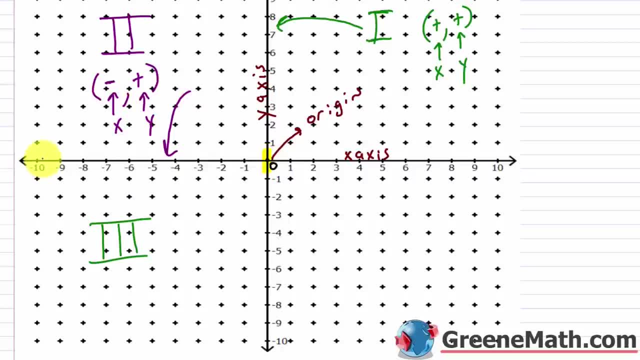 Now, in this quadrant, we're to the left of 0, so our x values are negative and we're below 0, so our y values are also negative. So again, this is my x values. these are my y values. 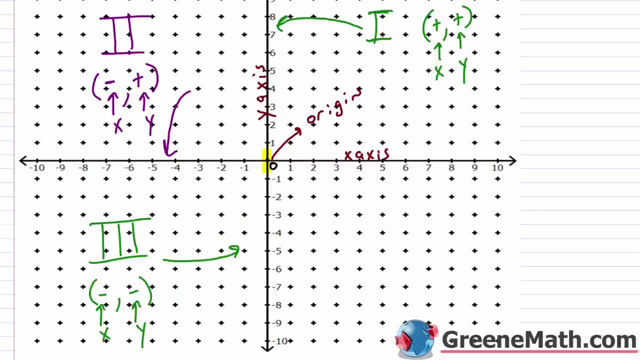 Alright, then the final quadrant. we go this way Again. it's counterclockwise, so it just goes this way. We end up here, and this is quadrant 4.. And in quadrant 4, the x values are to the right of 0, so they're positive. 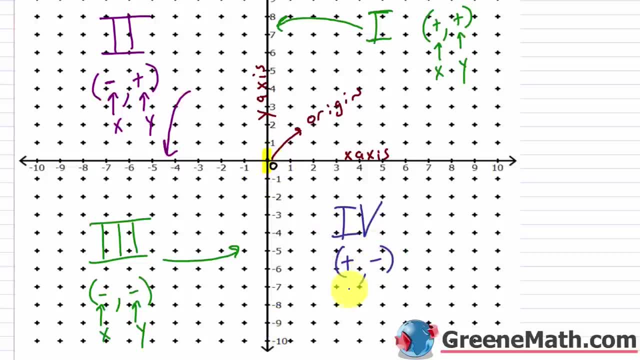 The y values are below 0, so they're negative. So this is the x values. These are the y values, So something you might want to write down. you might have a test and your teacher might say: what are the x values in quadrant 4?? 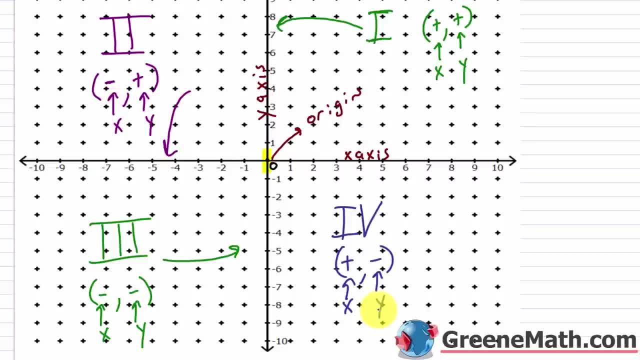 What are the y values in quadrant 4?? Are they positive or negative? Or she might give you an ordered pair and say what quadrant does it lie in? And if you've memorized the signs for each quadrant, you'll be able to tell right away. 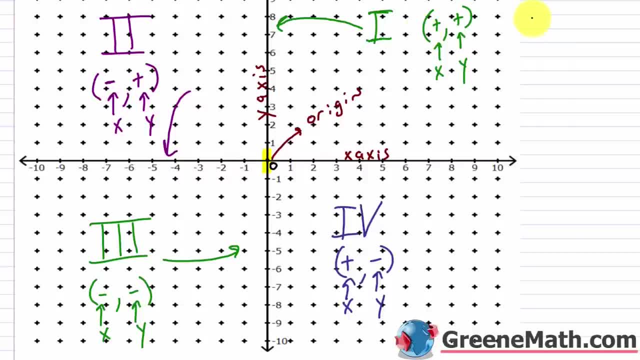 For example, if I gave you an ordered pair and that ordered pair was, let's say, 6 comma negative 3. Well, I know my x value has to be positive, so that can only be in quadrant 1 or 4.. 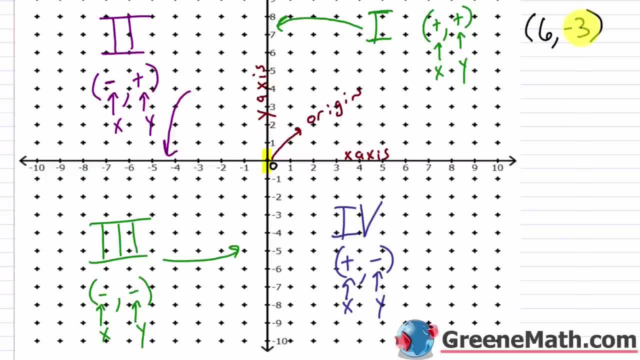 And the y value has to be negative. that can only occur in 4 or 3.. Now what fits both? Well, the x value is positive, the y value is negative, So that's quadrant 4.. X value is positive, y value is negative. 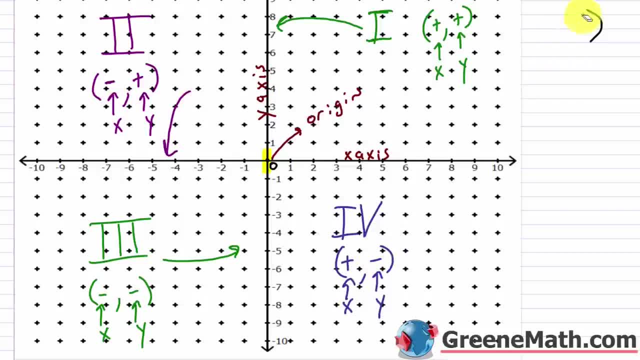 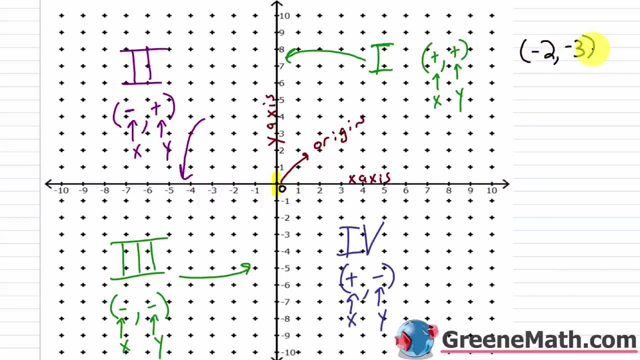 So this would be in quadrant 4.. Let's say, I gave you negative 2 comma, negative 3. It said: what quadrant is that in? Well, if we look here, this is negative and this is negative. So that occurs in the third quadrant, right. 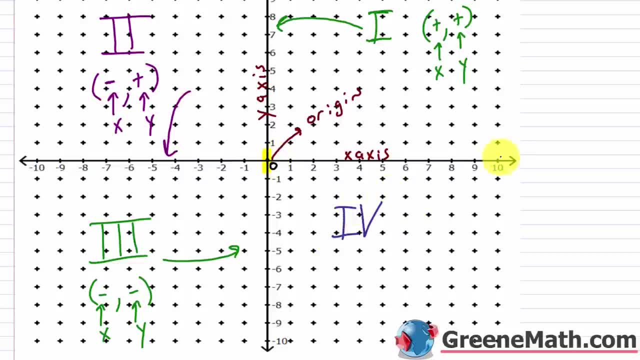 And in quadrant four, the x values are to the right of zero so they're positive. The y values are below zero so they're negative. 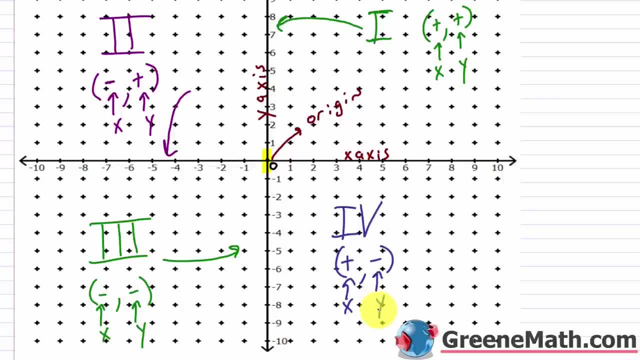 So this is the x values. These are the y values. So something you might 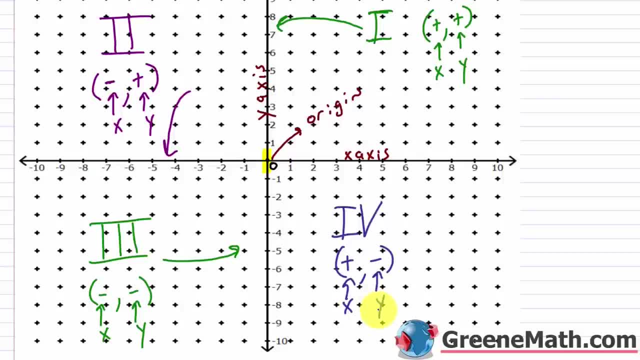 want to write down. You might have a test and you're going to have a teacher might say, 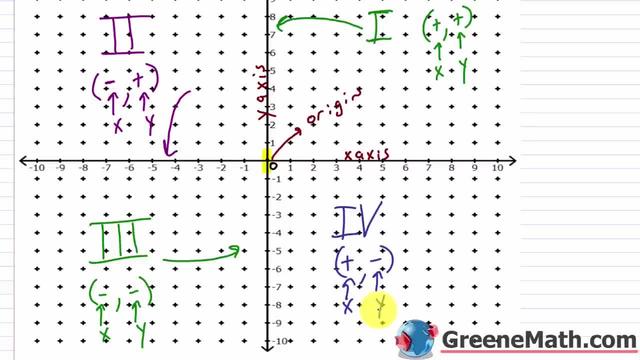 what are the x values in quadrant four? What are the y values in quadrant four? 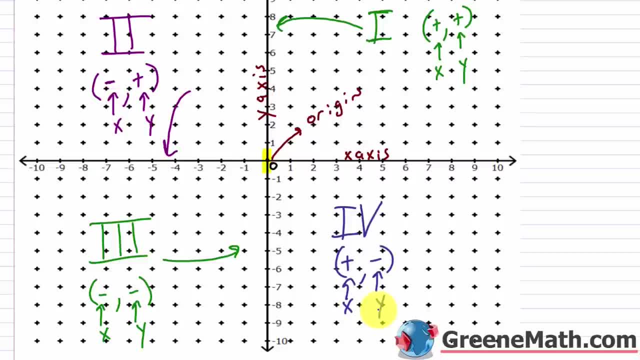 Are they positive or negative? Or she might give you an ordered pair 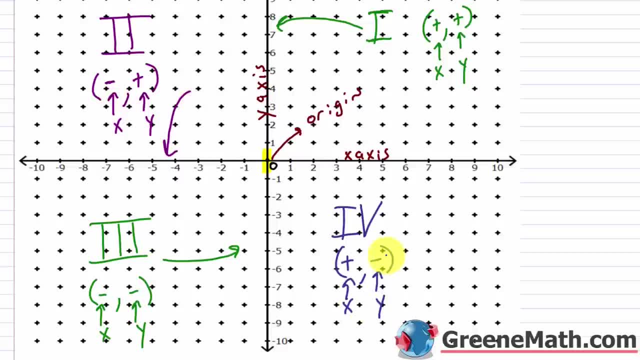 and say, what quadrant does it lie in? And if you've memorized 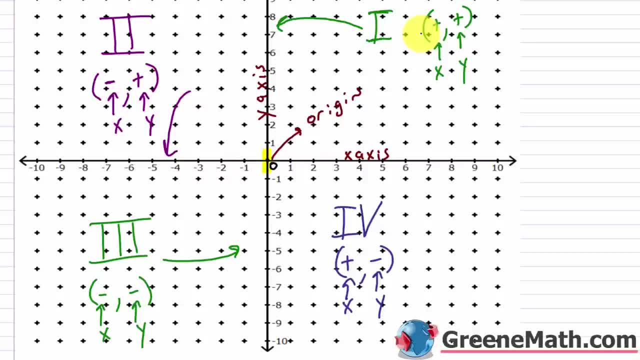 the signs for each quadrant, you'll be able to tell right away. For example, if I gave you an ordered pair 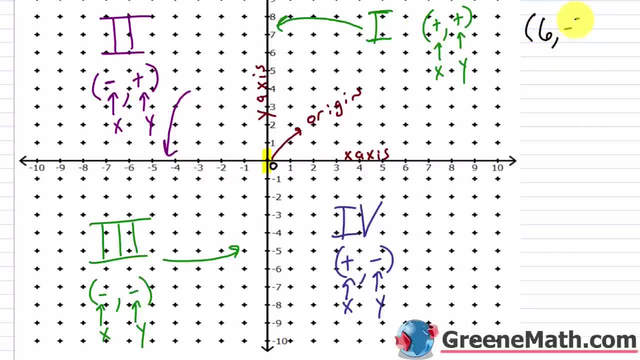 and that ordered pair was let's say six comma negative three, well, I know my x value has to be positive so that can only be in quadrant one or four. And the y value has to be negative. That can only occur in four or three. Now what fits both? Well, the x value is positive, the y value is negative. 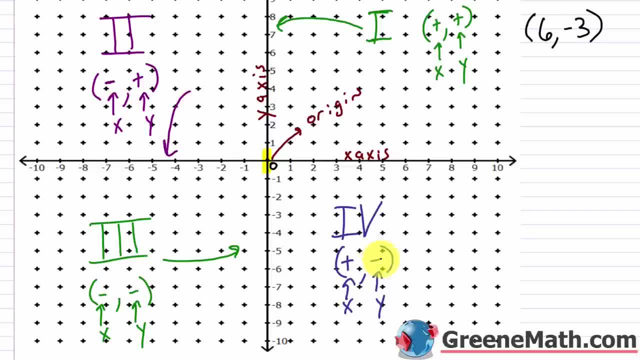 So that's quadrant four. x value is positive, y value is 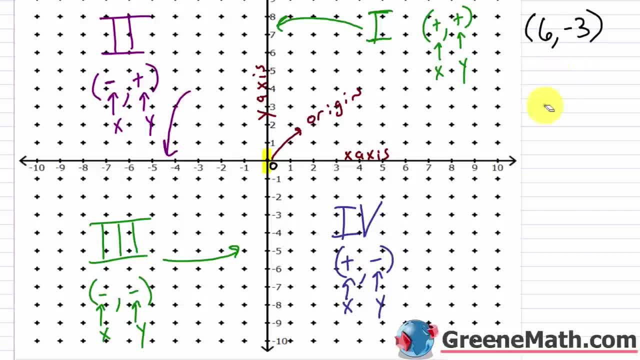 negative. So this would be in quadrant four. Let's 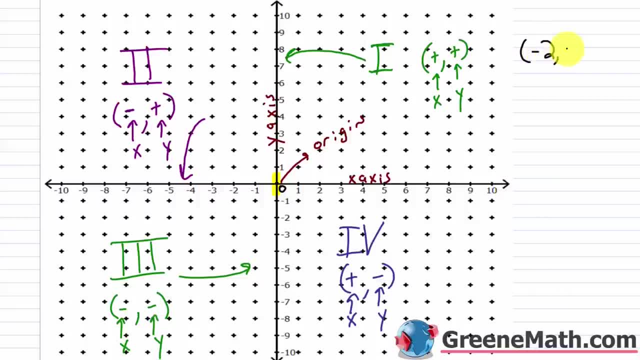 say I gave you negative two comma negative three. It said what quadrant is that in? Well, if we look here, this is negative and this is negative. 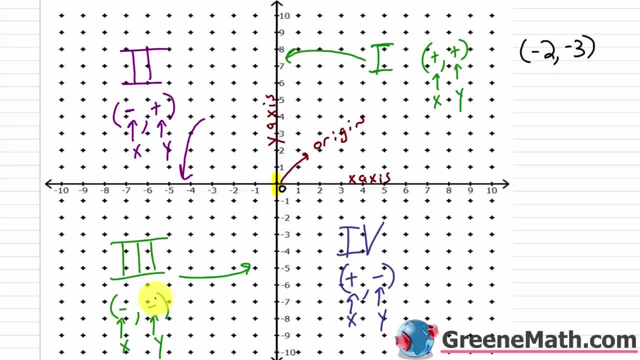 So that occurs in the third quadrant, right? Negative and negative. So then this is in the third quadrant. So not 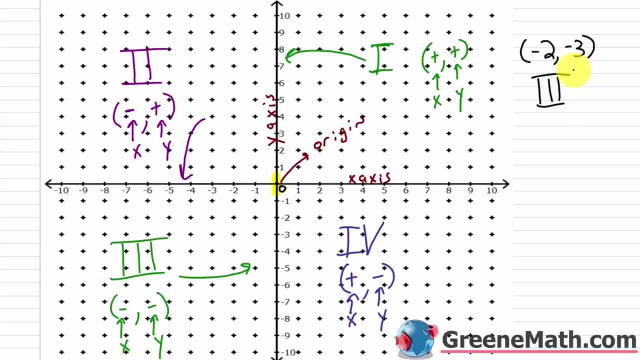 very difficult, just some basic memorization going on there. And something you might be tested on, so you might want to take note of that. Alright, so now let's talk about 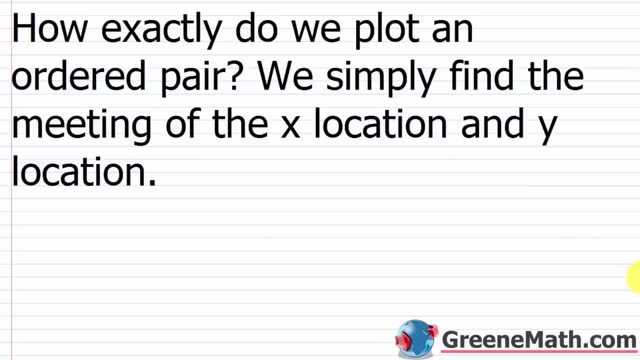 the main thing here. How exactly do we plot an ordered pair? Well, we simply find the meeting of the x location and y location. And I'm going to show you this through some examples. 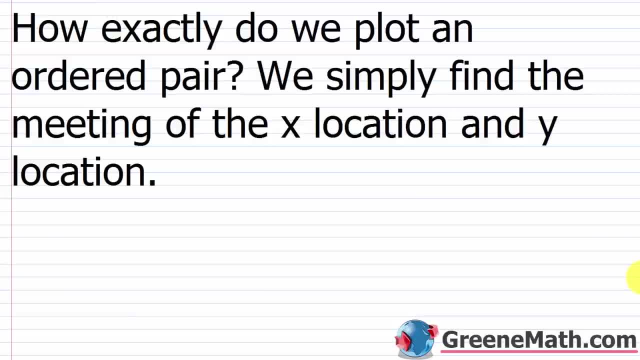 It's very, very easy. Once you do it a few times, you pretty much have the hang of it 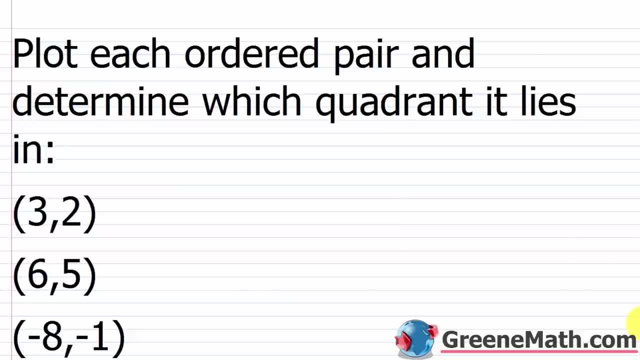 right away. So we want to plot each ordered pair and determine which quadrant it lies in. 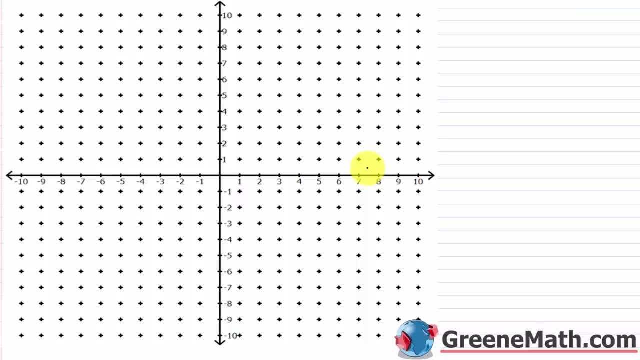 And I'm going to start out with three comma two. So we'll come down to our coordinate plane. Let me just write our ordered pair off to the side. Three comma two. And I just want to call your attention to a couple things. I want you to recall that this is the 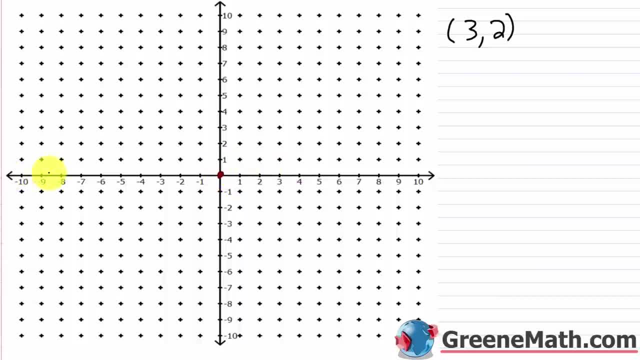 origin. Okay, this is the origin. The horizontal axis, the one that's going sideways, is the x-axis. This is your x-axis. Your vertical axis is the y-axis. So I'll label this one as x, this one as y. 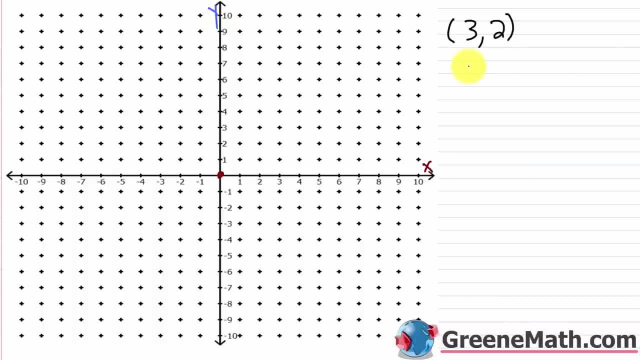 Now with your ordered pair, remember the left value is the x-value, the right value is the y-value. 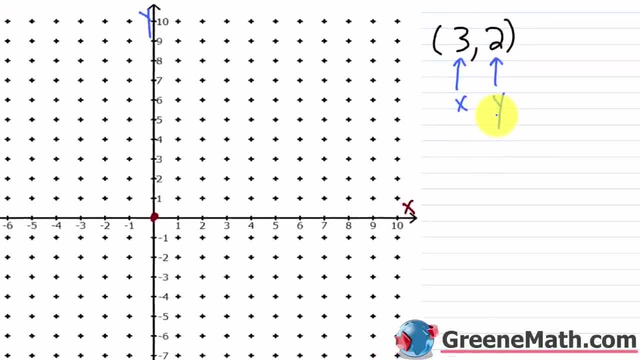 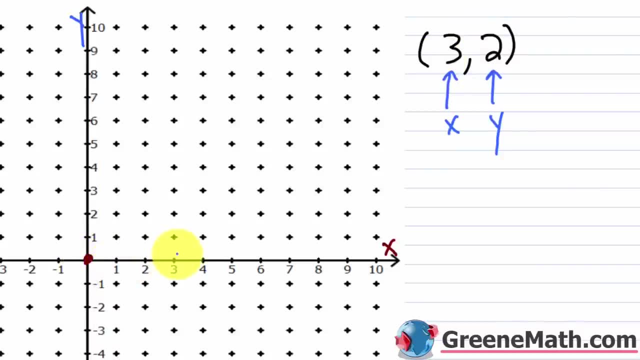 So, what I can do is I can start at the origin. If I have an x-value of three, that tells me to go three units to the right. So one, two, three units to the right. This is three. And then a y-value of two means I'm going up two units. So I'm going up one and then two. 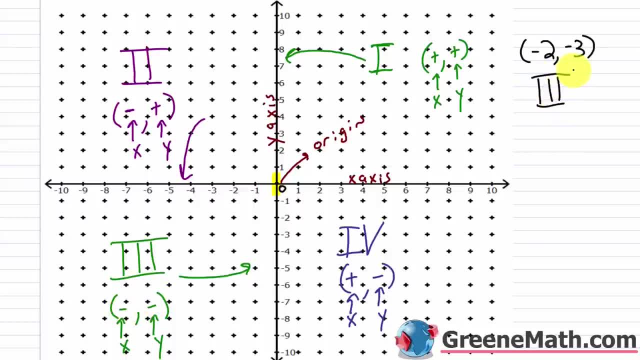 Negative and negative. So then this is in the third quadrant, So not very difficult, just some basic memorization going on there and something you might be tested on, so you might want to take note of that. All right, so now let's talk about the main thing here. 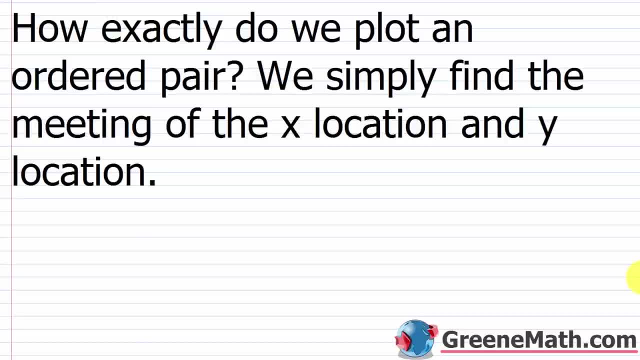 How exactly do we plot an ordered pair? Well, we simply find the meeting of the x location and y location, And I'm going to show you this through some examples. It's very, very easy. Once you do it a few times, you pretty much have the hang of it right away. 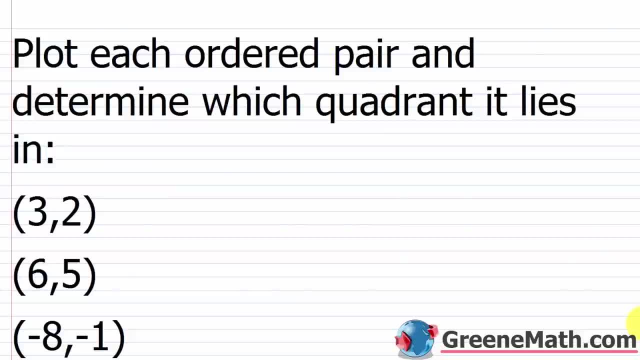 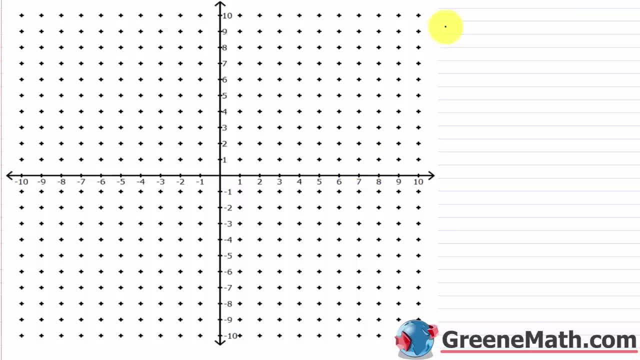 So we want to plot each ordered pair and determine which quadrant it lies in. And I'm going to start out with 3 comma 2.. So we'll come down to our coordinate plane. Let me just write our ordered pair off to the side 3 comma 2.. 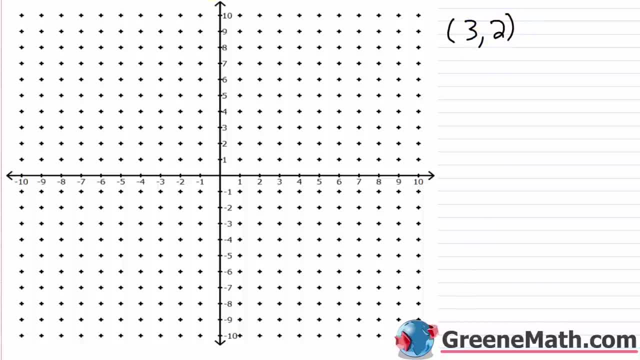 And I just want to call your attention to a couple of things. I want you to recall that this is the origin. Okay, This is the origin. The horizontal axis, the one that's going sideways, is the x axis. This is your x axis. 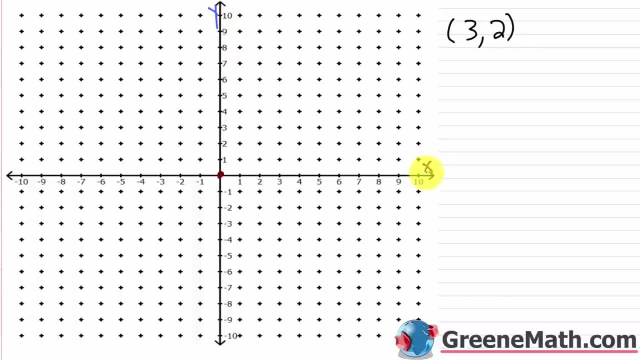 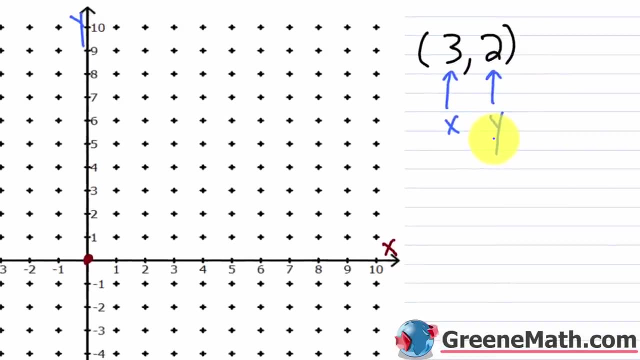 Your vertical axis is the y axis, So I'll label this one as x, this one as y. Now with your ordered pair. remember, the left value is the x value, the right value is the y value. So what I can do is I can start at the origin. 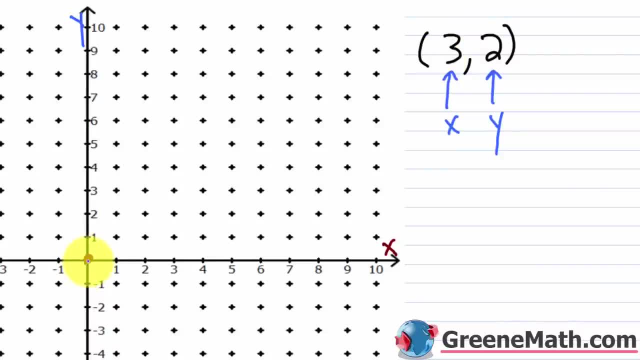 If I have an x value of 3, that tells me to go 3 units to the right. So 1, 2, 3. 3 units to the right, This is 3.. And then a y value of 2 means I'm going up 2 units. 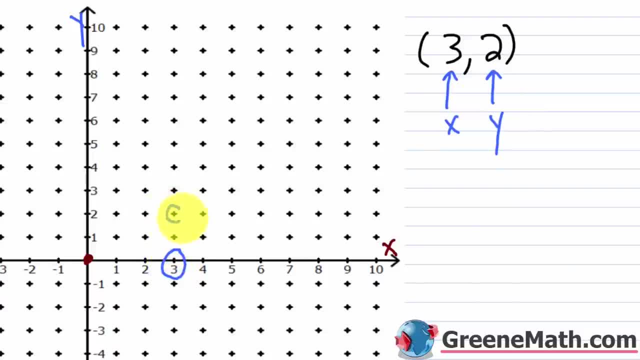 So I'm going up 1 and then 2.. So this would be the location 3, comma 2.. That's where that ordered pair would lie on the coordinate plane. Now, you could have done that a different way, And I'll just fill in that space. 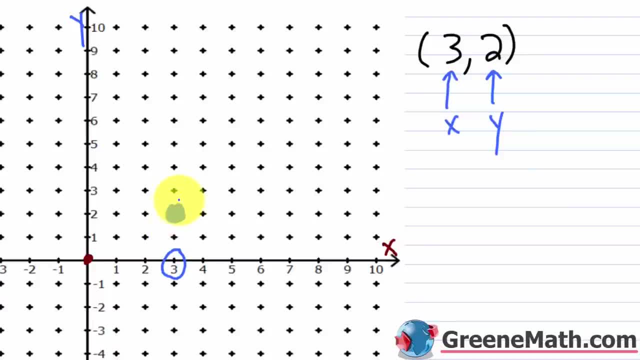 Kind of take your pencil or your pen and just kind of fill in a circle, Just like if you're filling in the answer on a Scantron Right. Just make a filled in circle, filled in dot. That's a little too big. 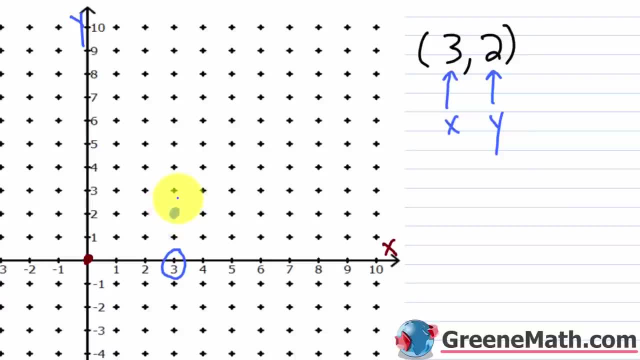 Let me make it a little bit smaller. Something like that. Now also, what I could have done is started at a y value of 2. So going up 1,, 2. And then went over to the right 3. So go over 1,, 2,, 3.. 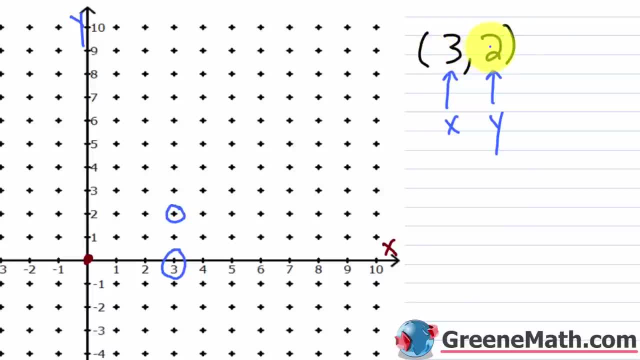 So this would be the location three comma two. That's where that ordered pair would lie on the coordinate plane. 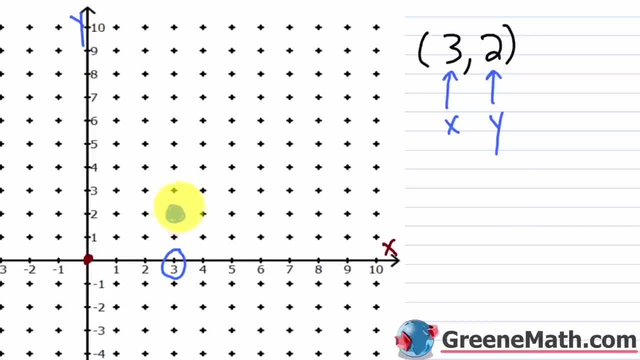 Now, you could have done that a different way. And I'll just fill in that space. 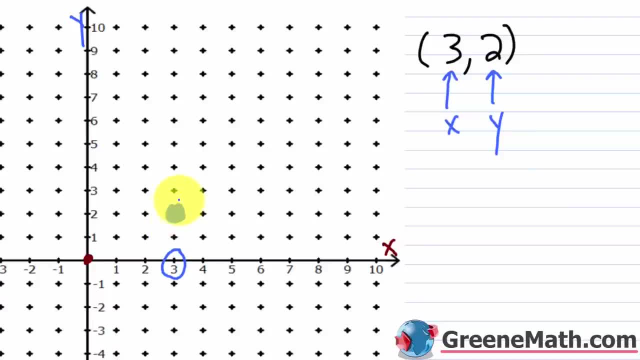 Kind of take your pencil or your pen and just kind of fill in a circle. Just like if you're filling in the answer on a Scantron. That's the same thing. Just make a filled in circle, filled in dot. 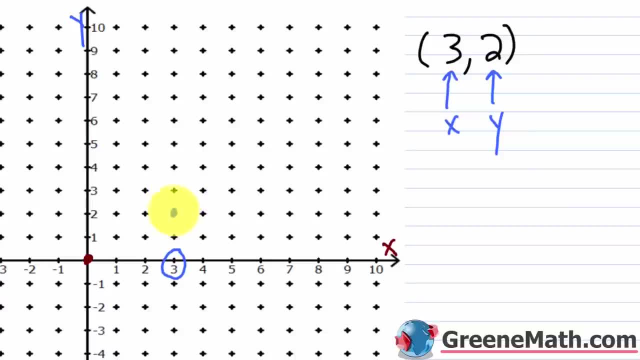 That's a little too big. Let me make it a little bit smaller. 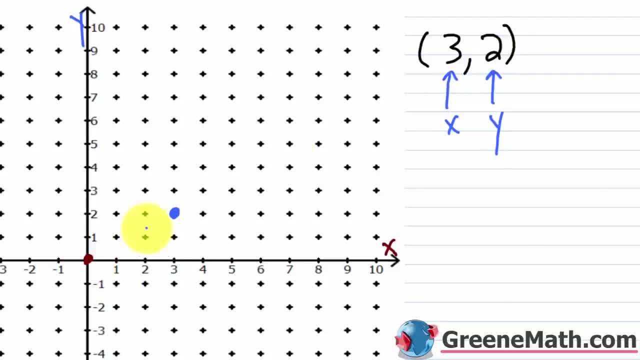 Now, also what I could have done is started at a y-value of two. So going up one, two. And then went over to the right three. So go over one, two, three. And again, I end up at the same spot. 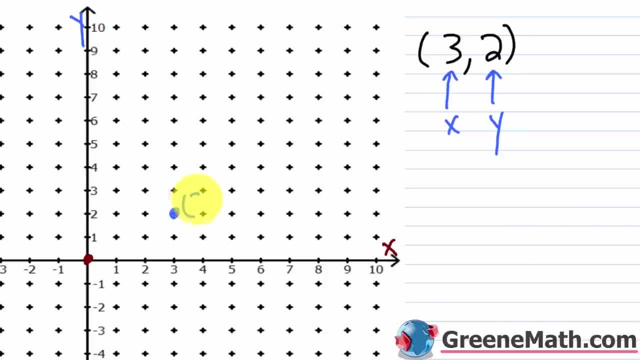 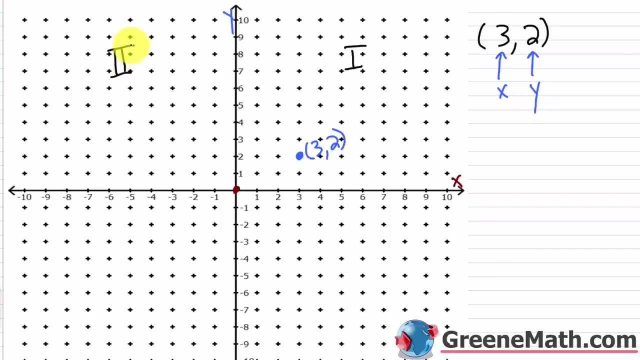 So whichever one you do first, you end up at the same spot. This is three comma two. And then it asks which quadrant does it lie in? Well, you remember the quadrants go like this. This is the first quadrant. And it goes counterclockwise. So it goes this way. This is the second. 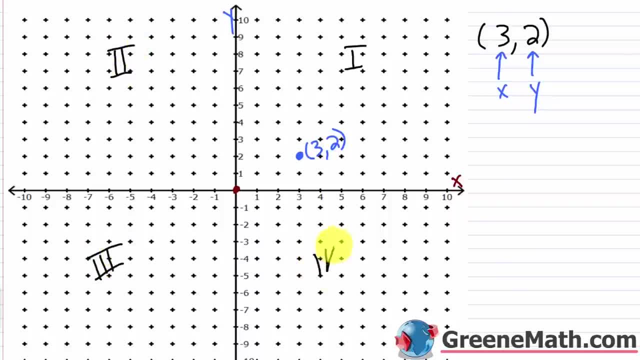 This is the third. And then this is the fourth. So this lies in the first quadrant. So this is quadrant number one. 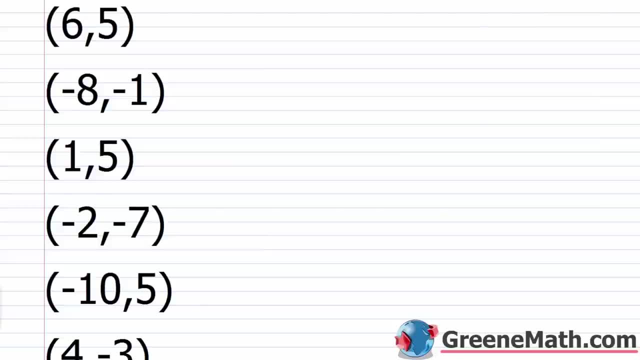 Alright, so our next ordered pair is six comma five. So now we're looking at six comma five. Again, this is your x-value. This is your 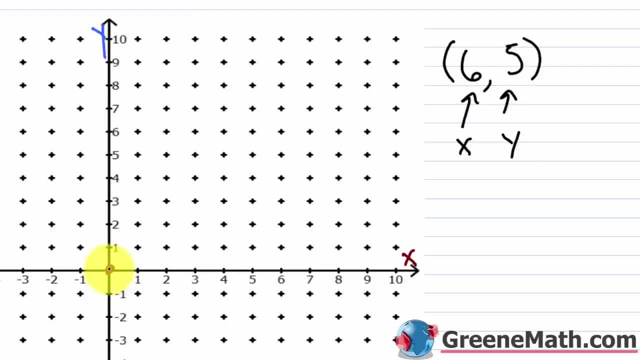 So I can start out at the origin and go six units to the right. This is six on the x-axis. And I want five on the y-axis. So I would just go five units up. So one, two, three, four, five. So that's right there. Let me use a different color here. 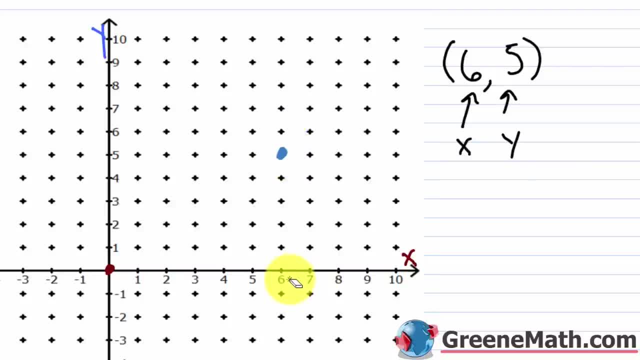 So that would be six comma five. And again, if you wanted to, you could start off at your y-location. So I could start off by starting at the origin and say I'm going up to five on the y-axis. So one, two, three, four, five. So that's right here. And then I could go over to the right six units. So one, two, three, four, five, six. 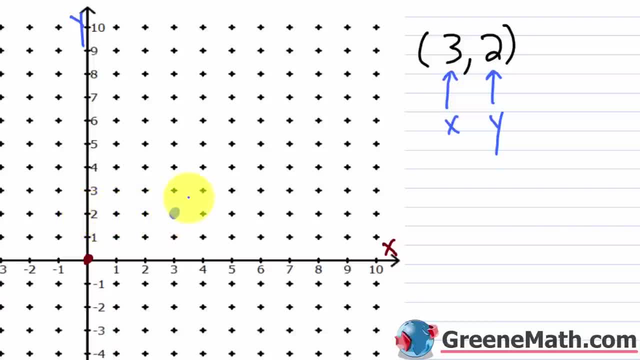 And again I end up at the same spot. So whichever one you do first, you end up at the same spot. This is 3 comma 2.. And then it asks: which quadrant does it lie in? Well, you remember, the quadrants go like this: 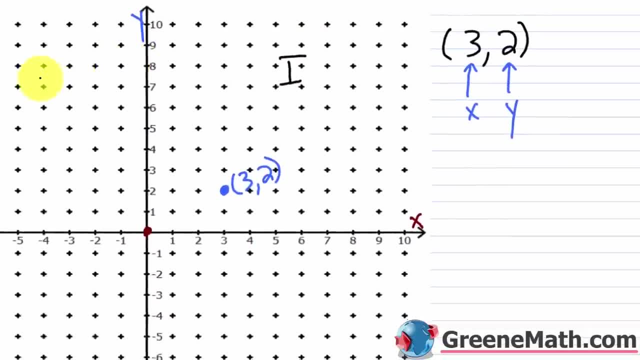 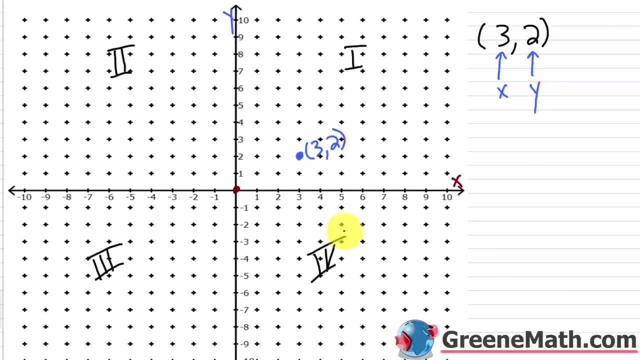 This is the first quadrant and it goes counterclockwise, So it goes this way. So this is the second, This is the third And then this is the fourth. So this lies in the first quadrant. This is quadrant number 1.. 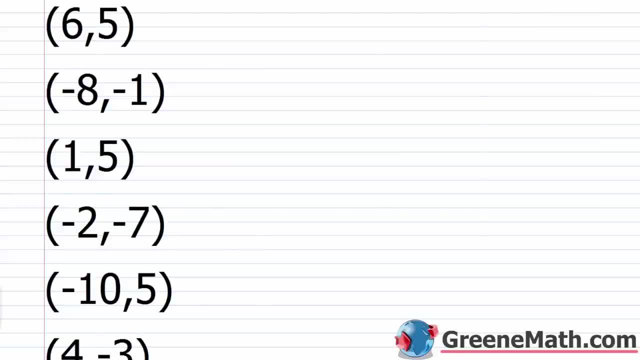 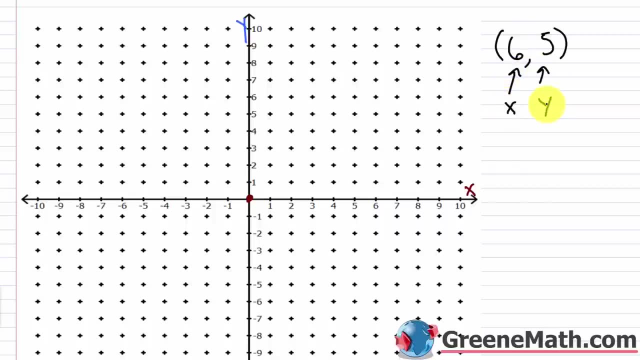 Alright, so our next ordered pair is 6 comma 5.. So now we're looking at 6 comma 5.. Again, this is your x value, This is your y value, So I can start out at the origin and go 6 units to the right. 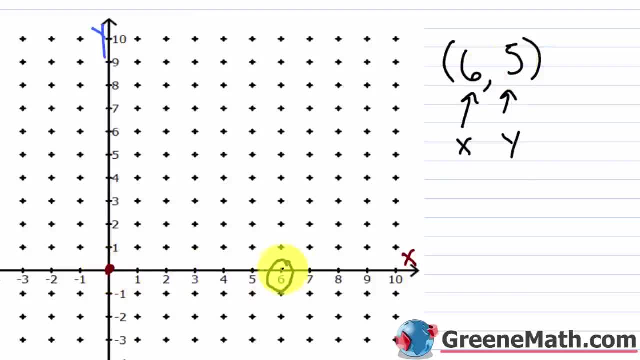 This is 6 on the x axis And I want 5 on the y axis, So I would just go 5 units up. So 1,, 2,, 3,, 4,, 5.. So that's right there. 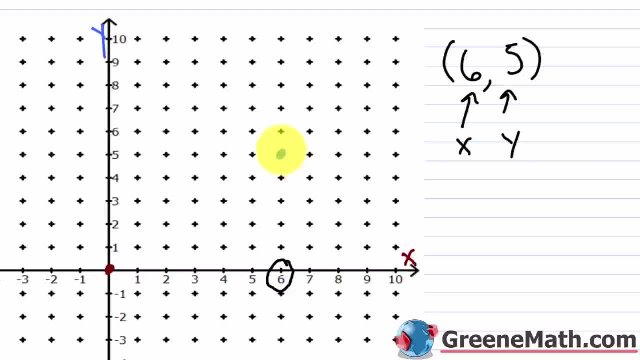 Let me use a different color here. So that would be 6 comma 5.. And again, if you wanted to, you could start off at your y location. So I could start off by starting at the origin. Say, I'm going up to 5 on the y axis. 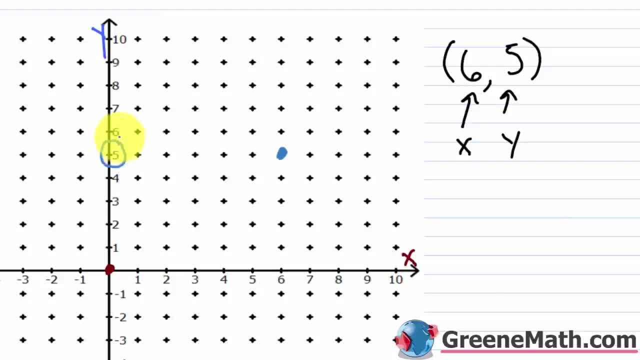 So 1,, 2,, 3,, 4, 5.. That's right here, And then I could go over to the right 6 units. So 1,, 2,, 3,, 4,, 5, 6.. 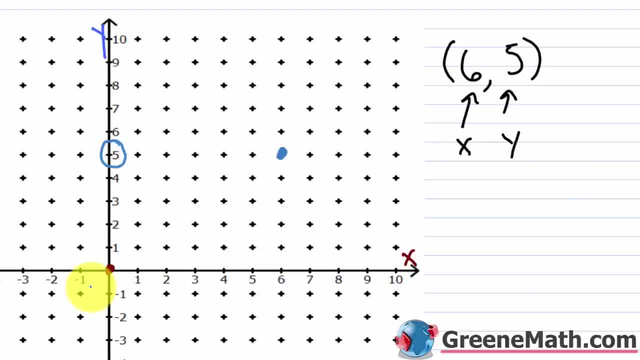 And I'm just counting for the sake of completeness. You can visually see where the intersection of 5 on the y axis and 6 on the x axis is. You can kind of pinpoint that. But again, when you first start you want to be completely sure. 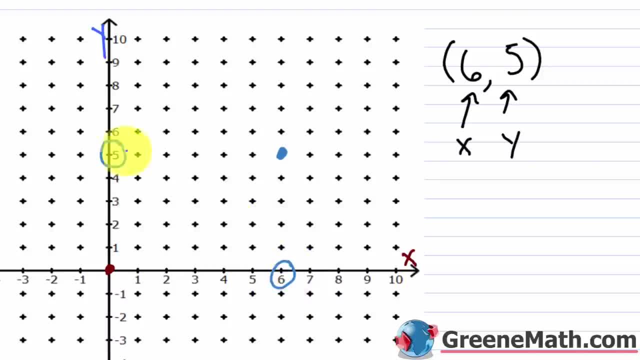 So you might want to say, okay, well, this is where 6 is on the x axis, This is where 5 is on the y axis, The intersection of the two. You know, You saw a little dotted line and that wasn't straight. 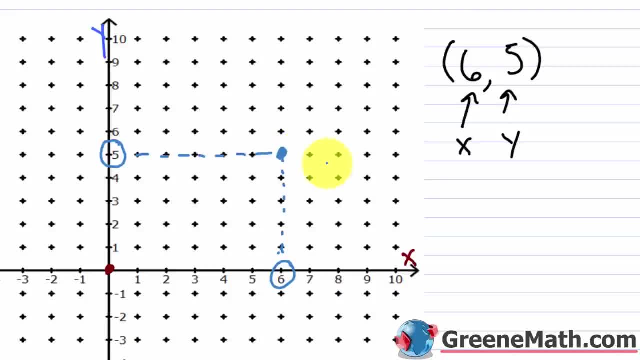 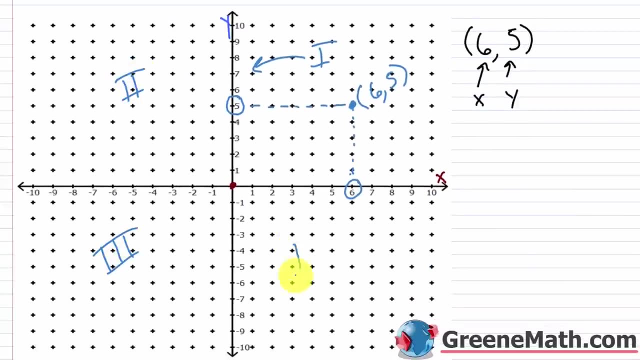 Right, And that's where they intersect. So this would be the point 6, comma 5.. And then, what quadrant is it in? Well, again, this is the first quadrant. Everything is positive, And it goes this way. This is the second quadrant, the third quadrant and the fourth quadrant. 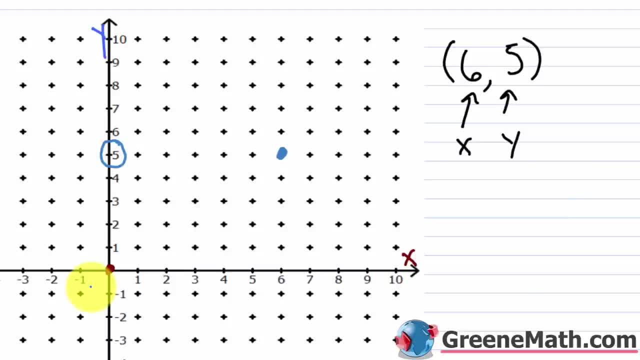 And I'm just counting for the sake of completeness. You can visually see where the intersection of five on the y-axis and six on the x-axis is. You can kind of pinpoint that. But again, when you first start, you want to be completely sure. So you might want to say, okay, well, this is where six is on the x-axis. This is where five is on the y-axis. 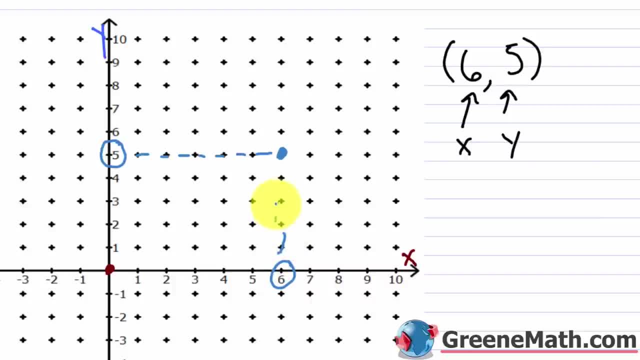 The intersection of the two, you can kind of draw a little dotted line. And that wasn't straight. 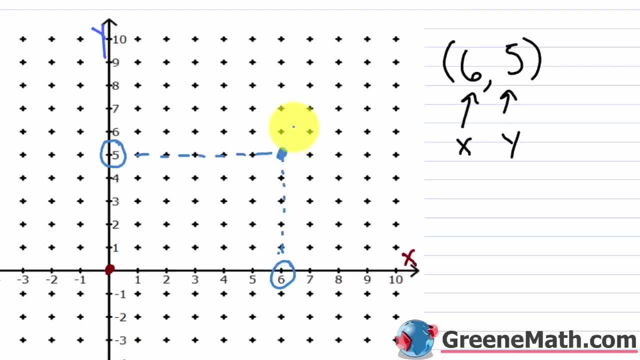 Alright, and that's where they intersect. So this would be the point six comma five. And then what quadrant is it in? Well, again, this is the first quadrant. Everything is positive. 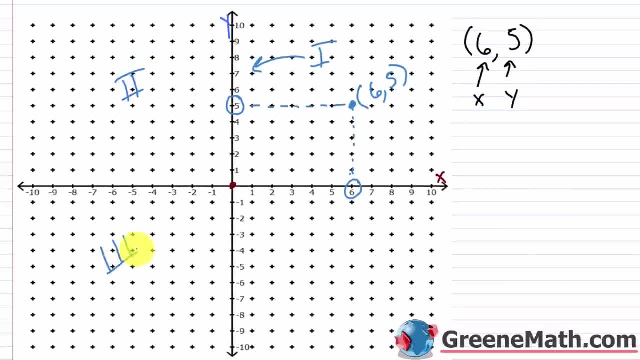 And it goes this way. This is the second quadrant, the third quadrant, and the fourth quadrant. 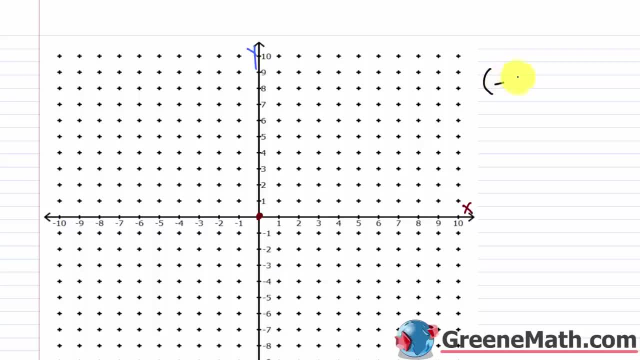 Alright, the next one is negative eight comma negative one. 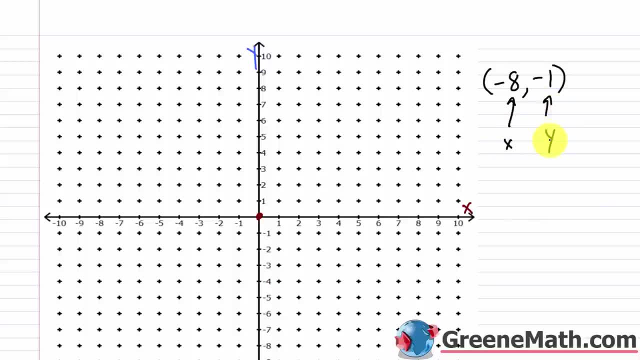 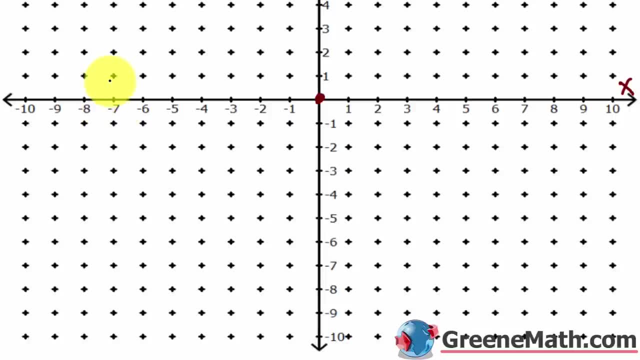 So again, this is your x location. This is your y location. And so I can start at the origin and I can go to the left eight units, find negative eight, or I can kind of make it quicker and just say, okay, the x location is negative eight. I can just start there. 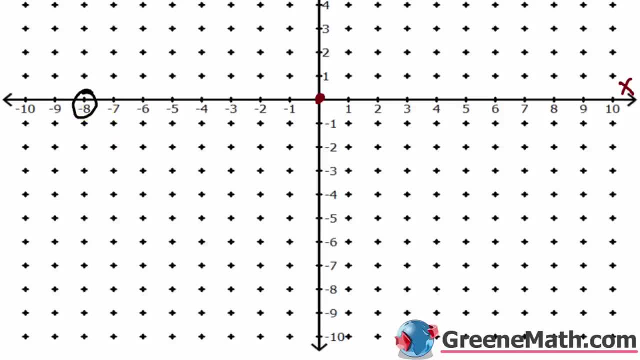 And my y location is negative one. So I would basically just go down one. And I would go down one. 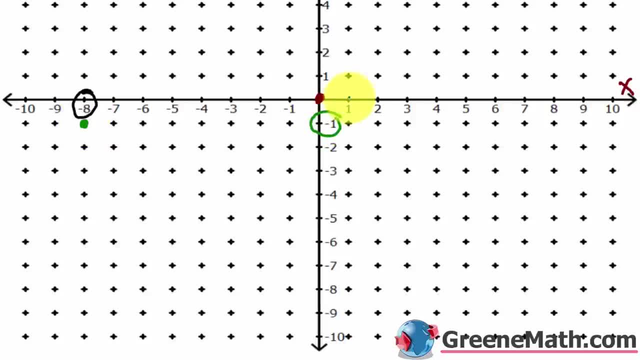 That's what I'm looking for. Here is negative one on the y-axis. 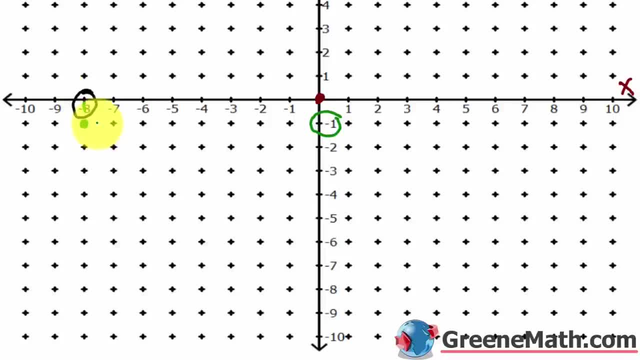 So you're looking again for where they meet. So you can kind of draw a 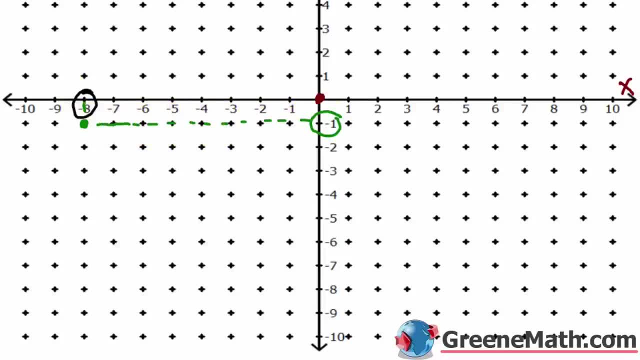 line for each. This is the meeting point. This is negative eight 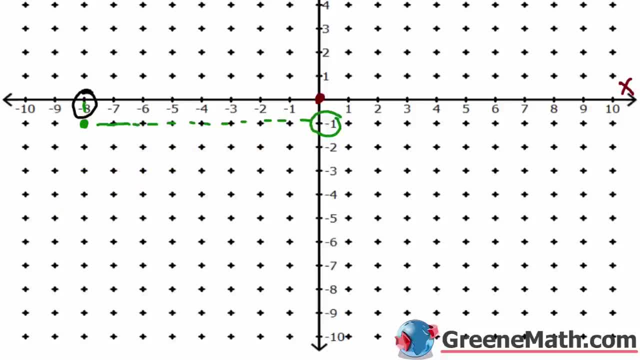 comma negative one. Let me do that in a different color. 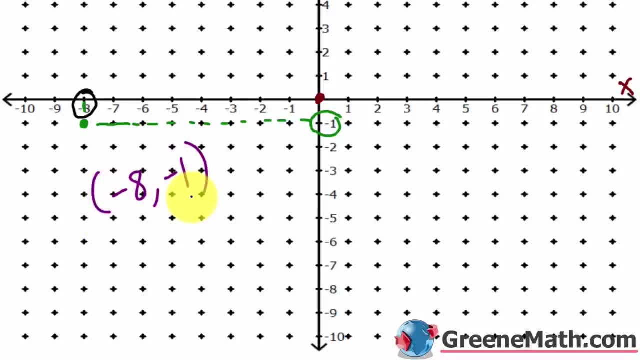 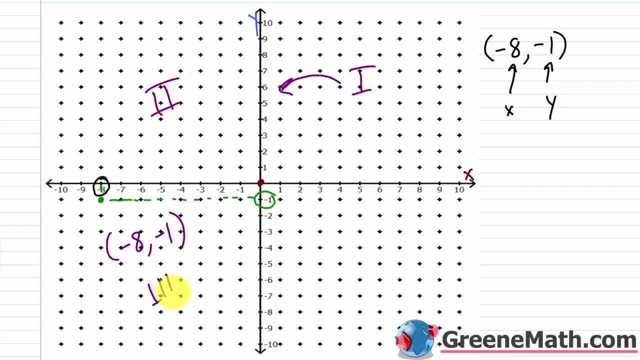 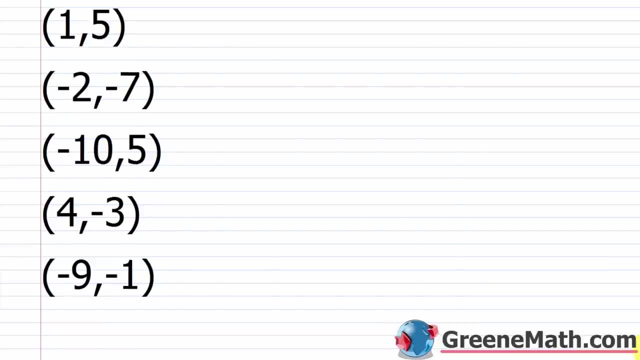 Negative eight comma negative one. And what quadrant does it lie in? Well again, this is the first. Move this way. This is the second. So then this would be the third. Alright, it lies in the third quadrant. And then for the sake of completeness, this is the fourth quadrant. Alright, what about one comma five? 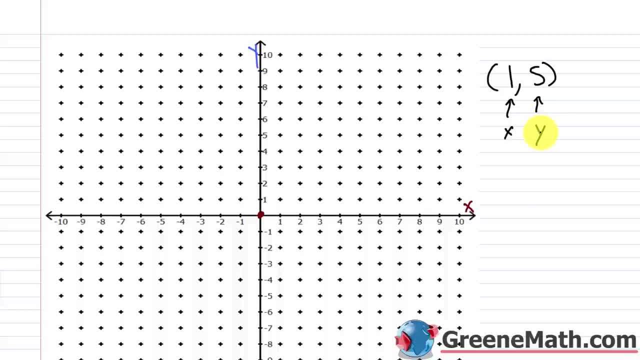 Again, my x location, my y location. 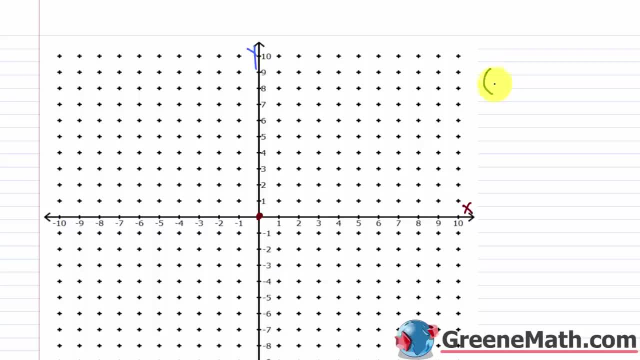 All right, The next one is negative 8 comma, negative 1.. So again, This is your x location, This is your y location, And so I can start at the origin And I can go to the left 8 units to find negative 8.. 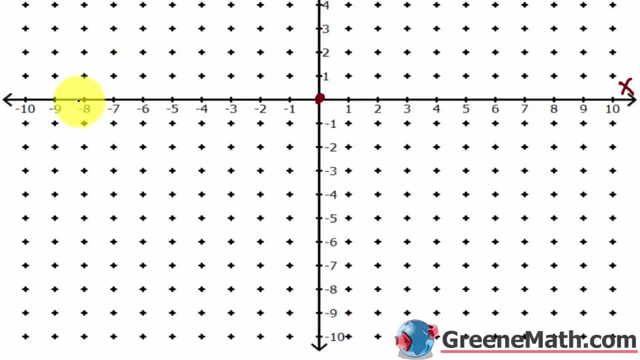 Or I can kind of make it quicker and just say: okay, the x location is negative 8. I can just start there, And my y location is negative 1. So I would basically just go down 1. And I would go down 1.. 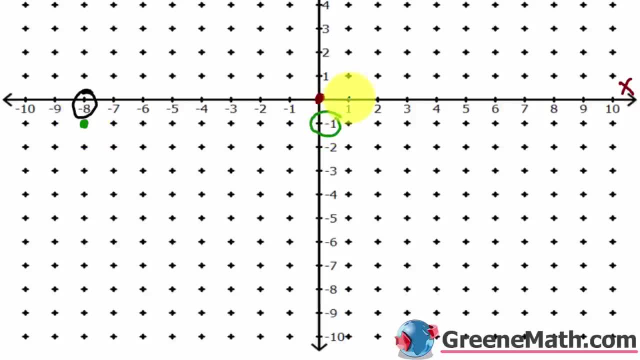 That's what I'm looking for Here- is negative 1 on the y axis. So you're looking again for where they meet, So you can kind of draw a line. You can draw a line for each. This is the meeting point. 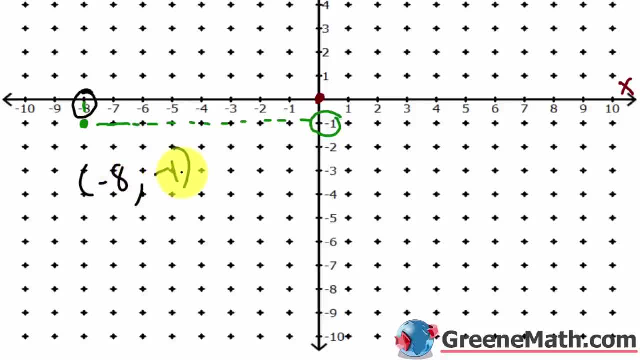 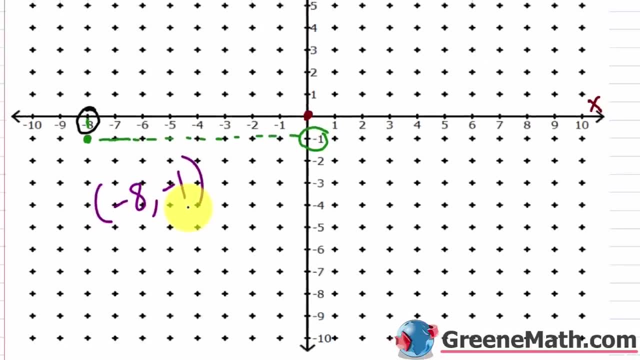 This is negative, 8 comma, negative, 1.. Let me do that in a different color: Negative, 8 comma, negative, 1.. And what quadrant does it lie in? Well, again, this is the first Move this way. This is the second. 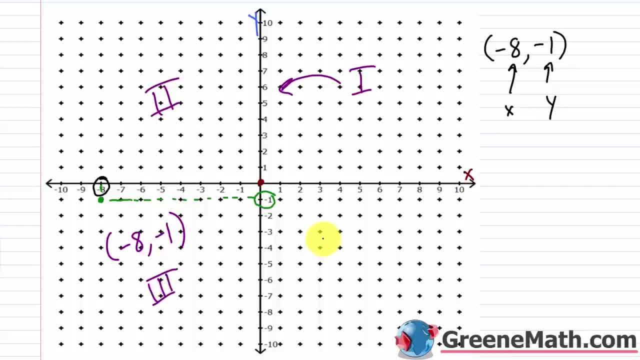 So then this would be the third. All right, It lies in the third quadrant. And then, for the sake of completeness, this is the fourth quadrant. All right, What about 1 comma 5?? All right, What about 1 comma 5?? 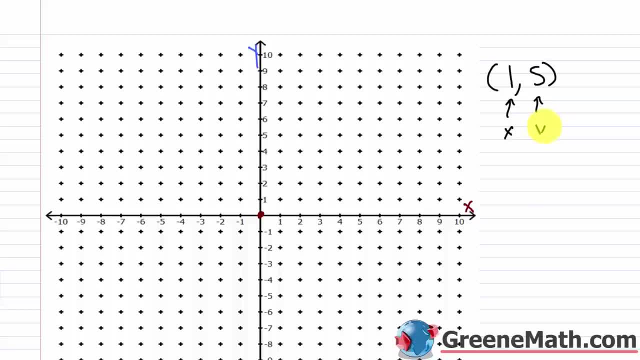 Again, my x location, my y location, So an x location of 1 and a y location of 5.. So let's kind of reverse it, Let's start out with the y location of 5.. So I would find that here. 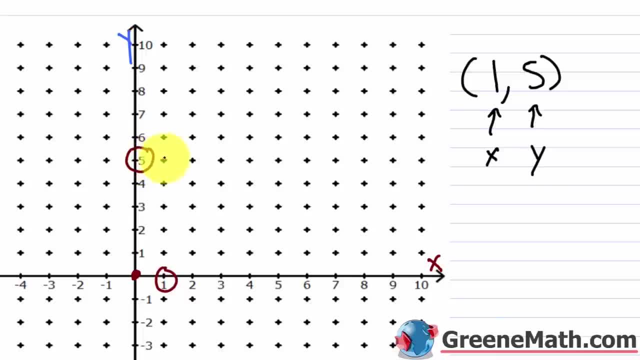 And an x location of 1 is here. So if I'm already up 5, I just need to go to the right 1.. Again, you can kind of draw a little line to see where they would intersect, And it's right there. 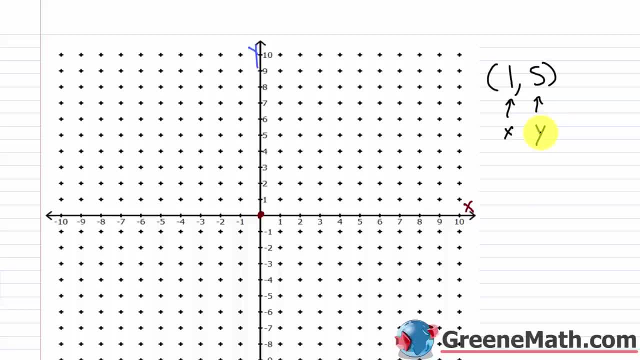 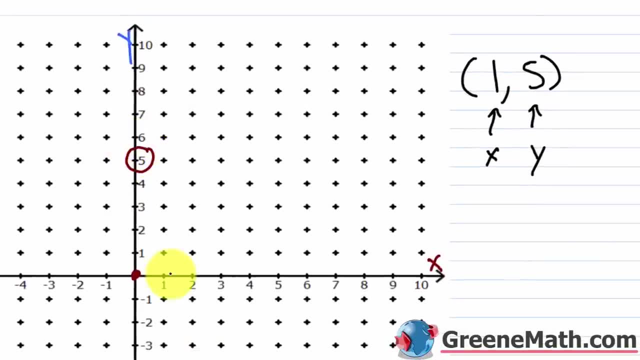 So an x location of one and a y location of five. So let's kind of reverse it. Let's start out with the y location of five. So I would find that here. And an x location of one is here. So if I'm already up five, I just need to go to the right one. Again, you can kind of draw a little line to see where they would intersect. 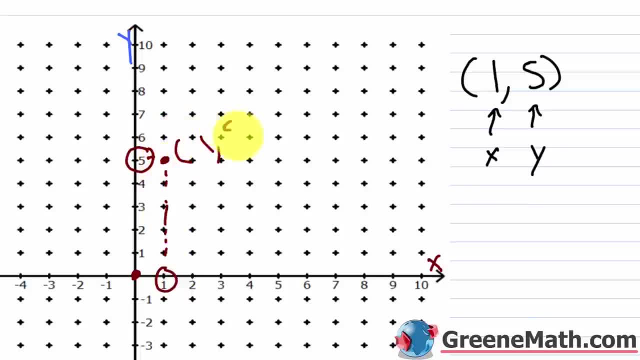 And it's right there. Alright, so this is one comma five. And this lies in the first three, four. 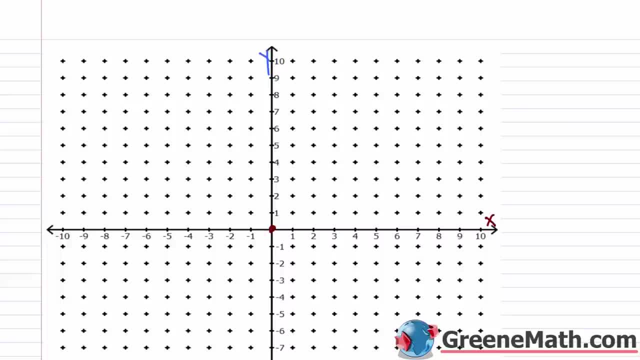 Alright, what about negative two comma negative seven? What about negative two comma negative seven? 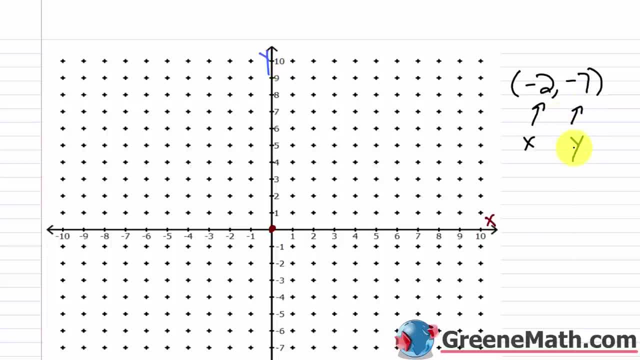 So this is the x value, this is the y value. 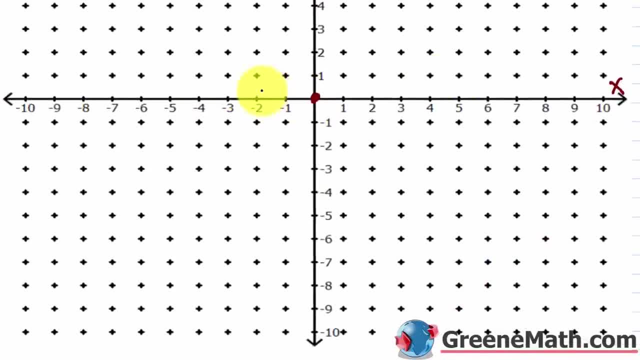 So an x value of negative two, if we're on the x axis, here's negative two. A y value of negative seven is here. So essentially 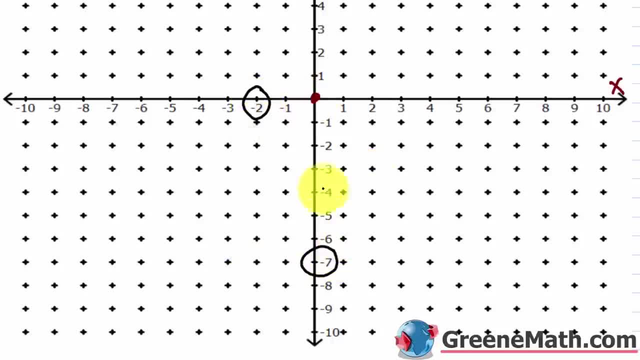 I'm going left two and down seven. Right? Or I'm going down seven and left two. It doesn't matter which order you kind of do this. Or you could start at negative two and just go down seven. 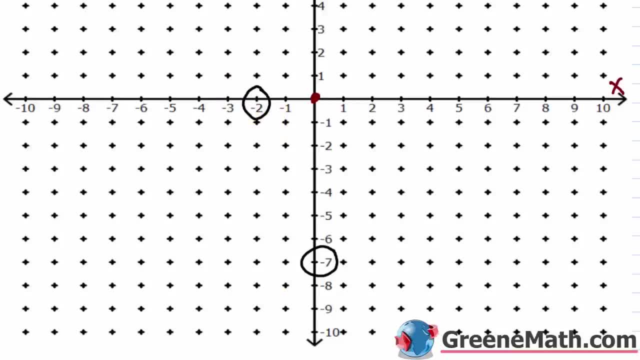 Again, a lot of different ways to do it. So if I want to, 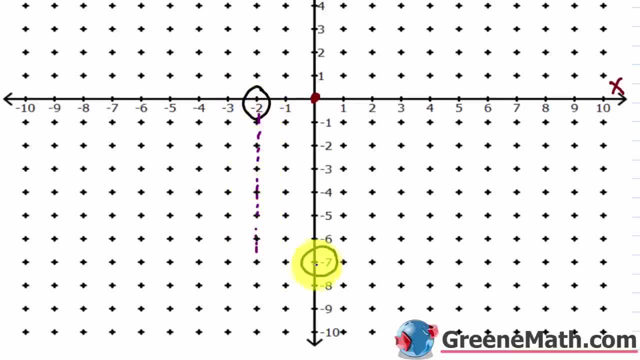 to make it completely clear, let me just draw a line there. Draw a line here. And that's my point. 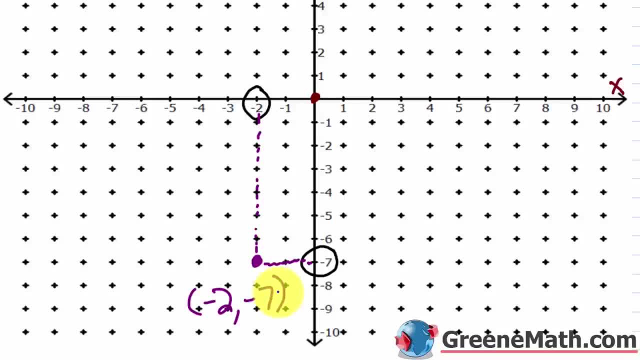 Alright, this is negative two comma negative seven. And which quadrant does a lie in? Again, this is the first one. 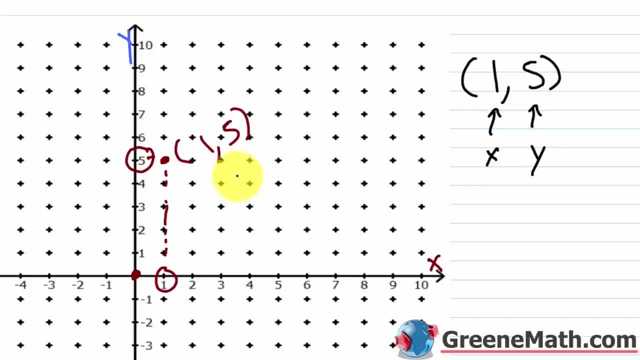 All right, So this is 1 comma 5.. And this line is negative: 1 comma 5.. All right, So this is the first quadrant. So this is the first quadrant. All right, 1,, 2,, 3, 4.. 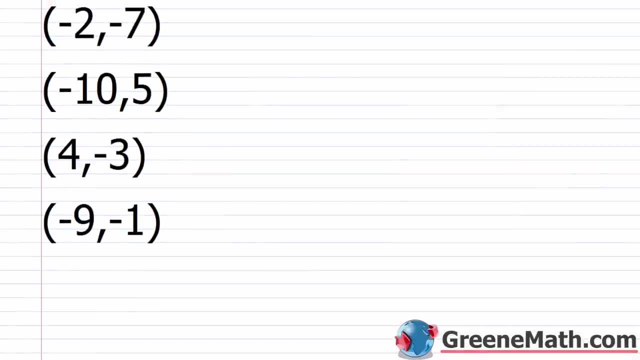 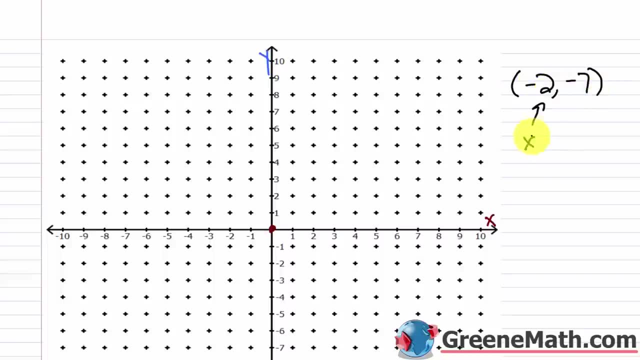 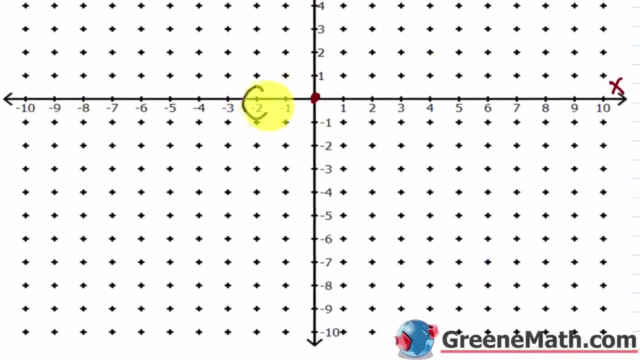 All right. What about negative 2 comma negative 7?? What about negative 2 comma negative 7?? So this is the x value, This is the y value. So an x value of negative 2, if we're on the x axis, here's negative 2.. 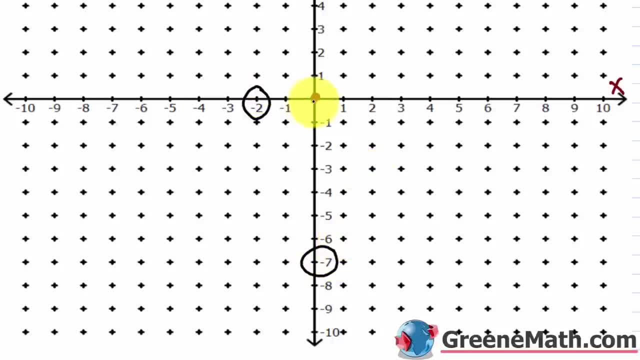 A y value of negative 7 is here. So essentially I'm going left 2 and down 7.. Right Down 7 and left 2.. It doesn't matter which order. you kind of do this, Or you could start at negative 2 and just go down 7.. 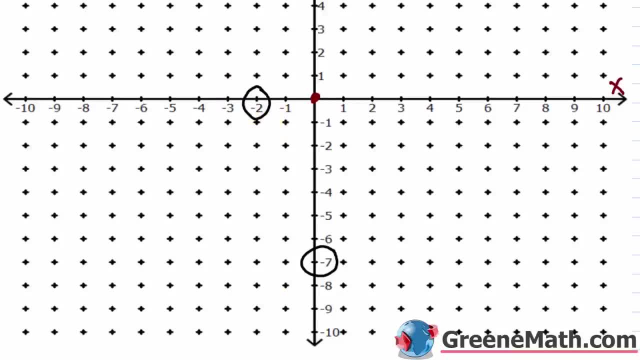 Again, a lot of different ways to do it. So if I want to, to make it completely clear, I'll just draw a line there, draw a line here, And that's my point. All right, This is negative 2 comma, negative 7.. 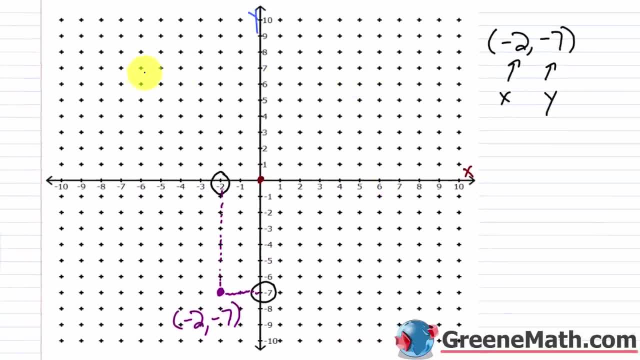 And which quadrant does a line? Again, this is the first one, This is the second one, This is the third one. So this is lying in the third quadrant And this is the fourth one. All right, It's counterclockwise. 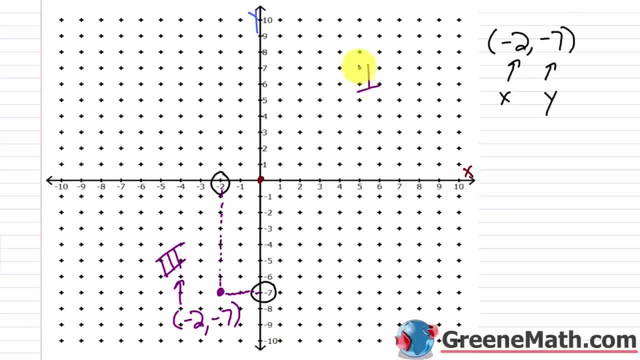 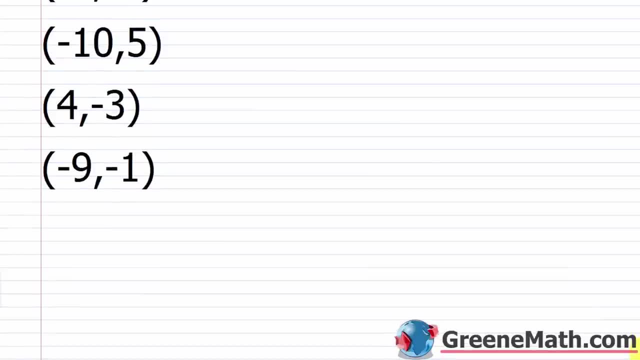 Just remember that it starts positive, positive, So it starts here And it goes this way: 1,, 2,, 3,, 4.. All right, So the next one is negative, 10 comma 5.. All right, So negative, 10 comma 5.. 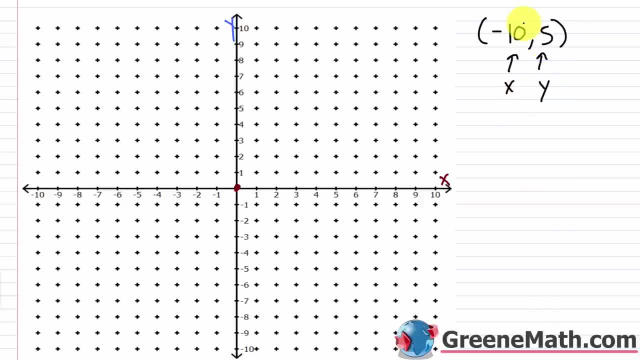 This is an x value. This is a y value, All right. So I'm going to find negative 10 on the x axis. That's all the way over here. I'm going to find 5 on the y axis, All right. 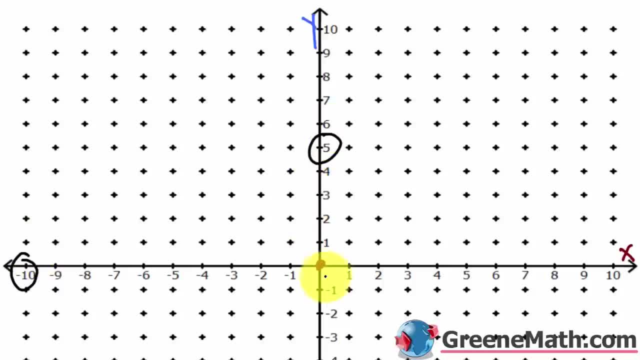 I'm going to find 5 on the y axis. That's right here. I'm just looking for their point of intersection, So I can go to the left 10 and up 5, or I can go up 5 and to the left 10.. 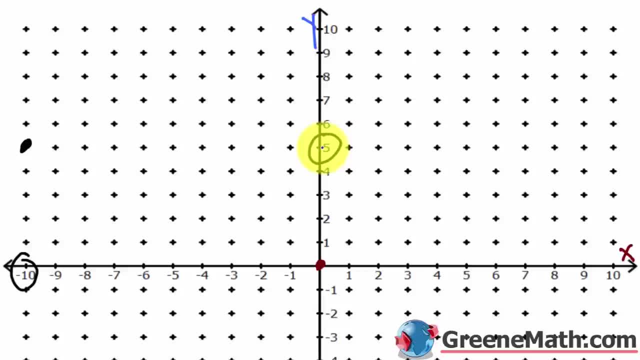 Again, it doesn't matter. All right, I could start out at 5 on the y axis and go over 10, or I could start out at negative 10 and go up 5.. However you do it, you're going to arrive at the same location, which is negative 10. 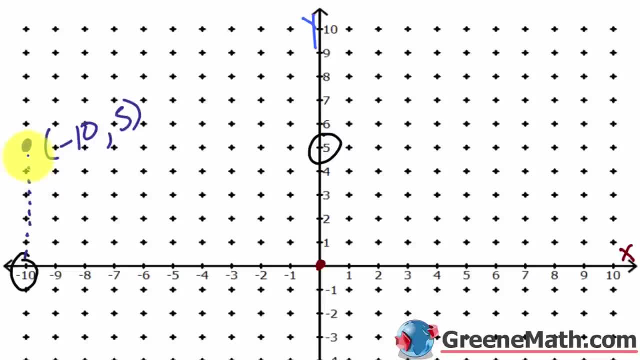 comma 5.. And again, if I want to just kind of draw a line like that and then another one like that to make it clear where they intersect, And then what quadrant is this? in? Well, this is the first quadrant and it goes counterclockwise. 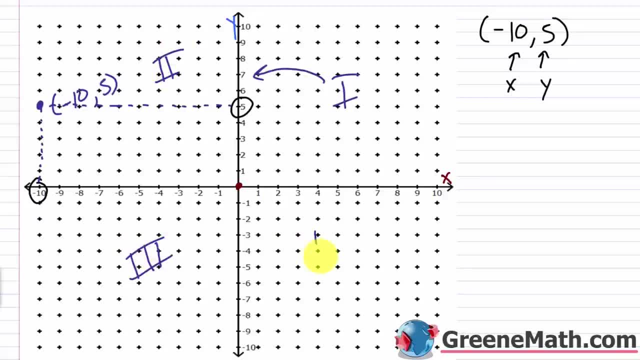 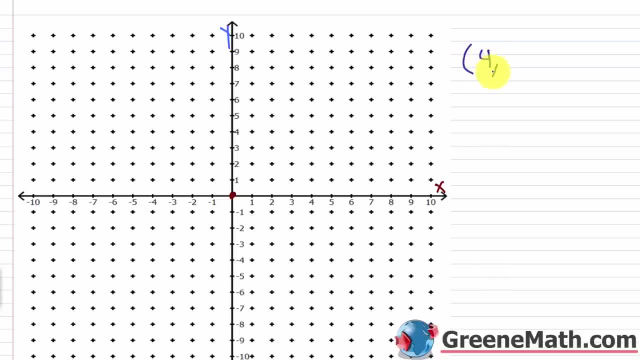 So this is number 2,, this is number 3, and again this is number 4.. So it's in the second quadrant, All right. So now we have 4 comma negative 3.. So 4 comma negative 3.. 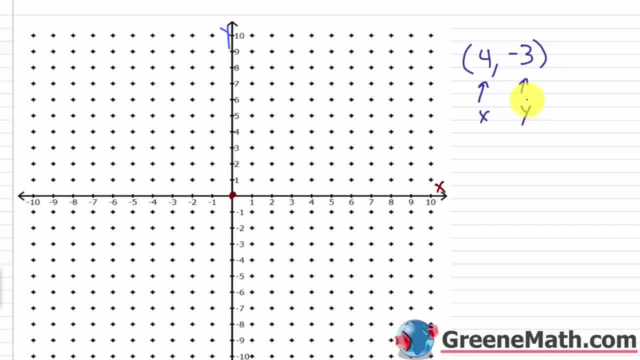 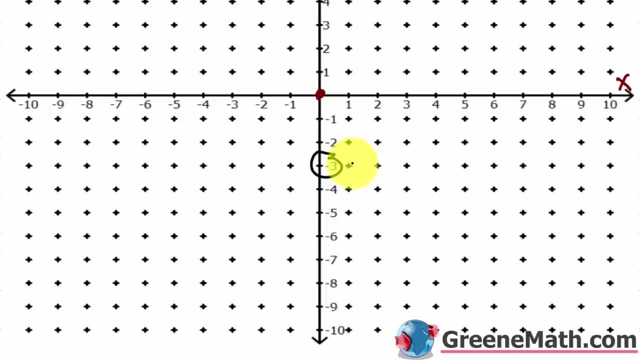 Again, this is the x value, This is the y value. So let's start out at negative 3 on the y axis. So let's start out here. Let's move 4 units to the right, The x axis, So 1,, 2,, 3,, 4.. 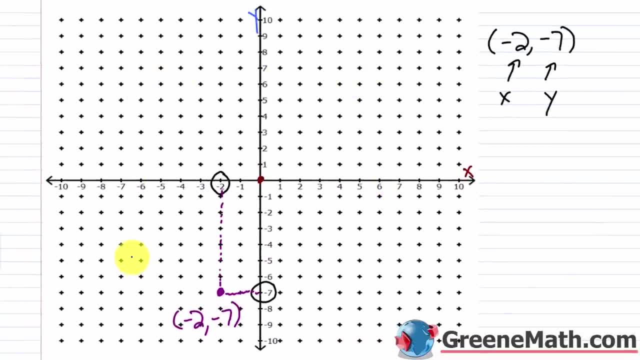 This is the second one. This is the third one. So this is lying in the third quadrant. 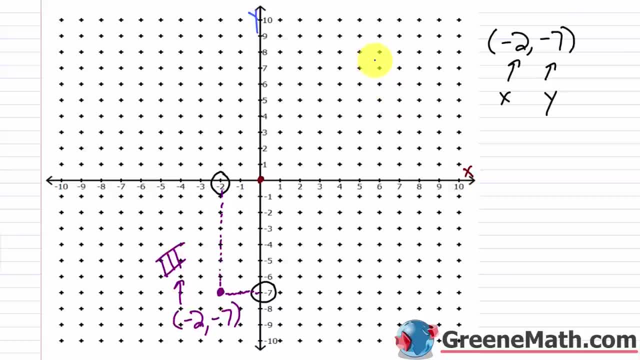 And this is the fourth one. Alright, it's counterclockwise. Just remember that it starts positive positive. 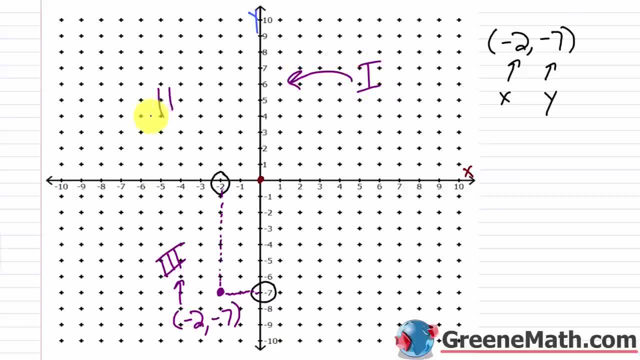 So it starts here. And it goes this way. One, two, three, four. Alright, so the next one is negative ten comma five. 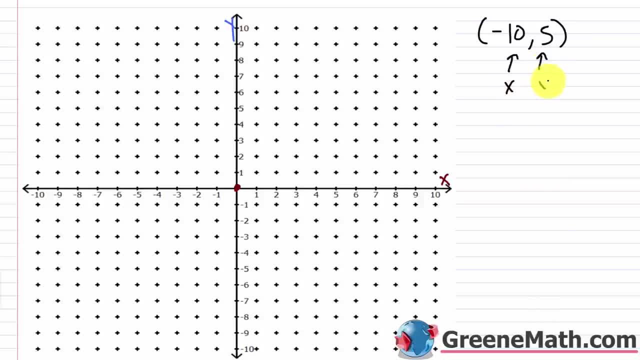 This is an x value. This is a y value. 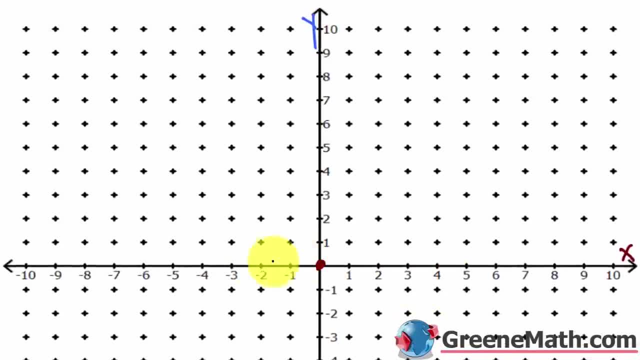 Alright, so I'm going to find negative ten on the x axis. That's all the way over here. I'm going to find five on the y axis. That's right here. I'm just looking for their point of intersection. 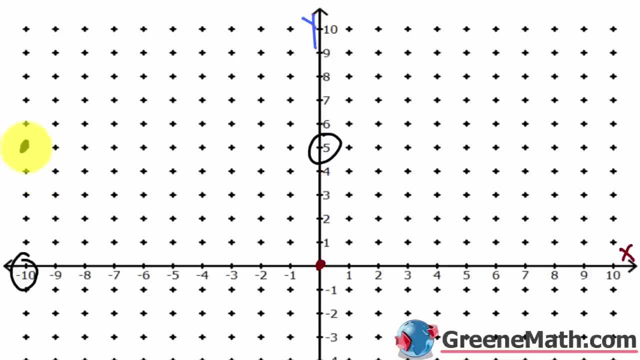 So I can go to the left ten and up five. Or I can go up five and to the left ten. 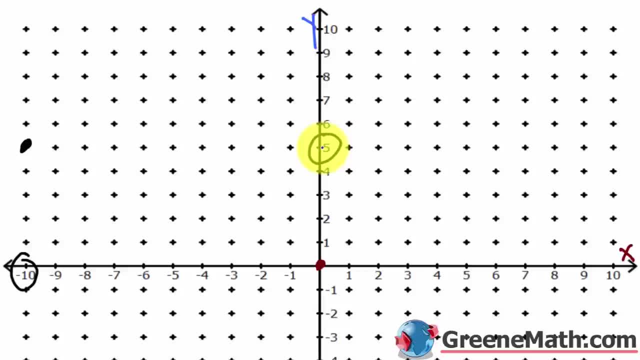 Again, it doesn't matter. Alright, I could start out at five on the y axis and go over ten. Or I could start out at negative ten and go up five. However you do it, you're going to arrive at the same 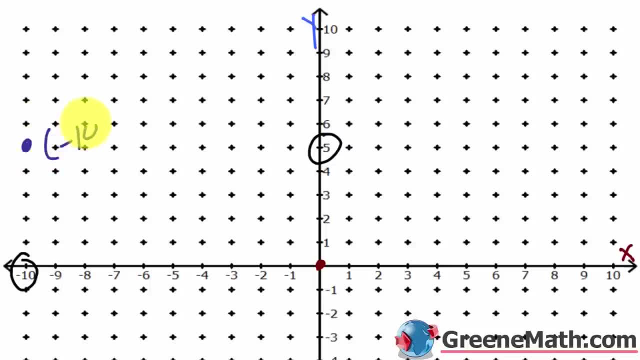 location. Which is negative ten 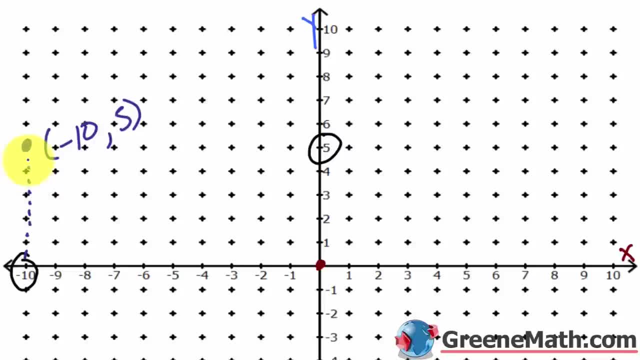 comma five. And again, if I want to just kind of draw a line like that. And then another one like that. To make it clear 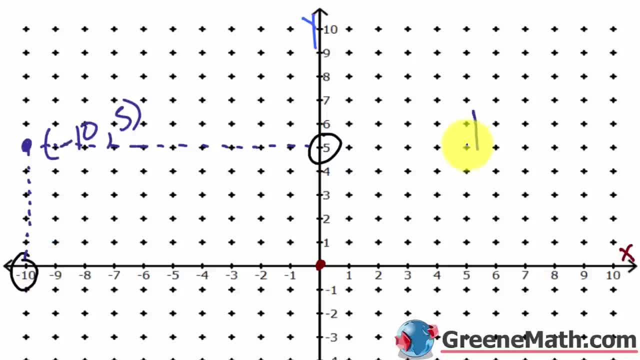 where they intersect. And then what quadrant is this in? Well, this is the first quadrant. And it goes counterclockwise. So this is number two. 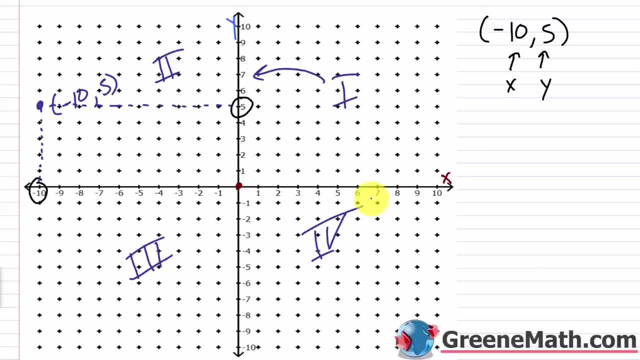 This is number three. And again, this is number four. 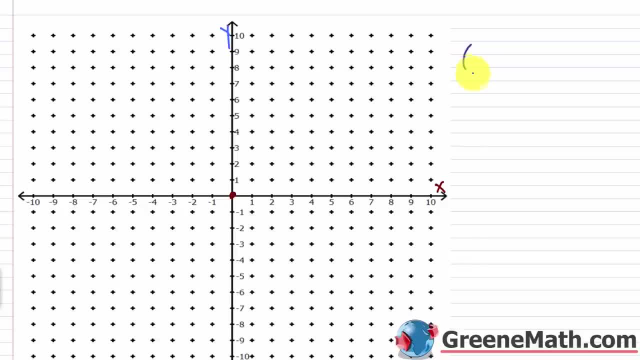 So it's in the second quadrant. Alright, so now we have four comma negative three. So four comma negative three. 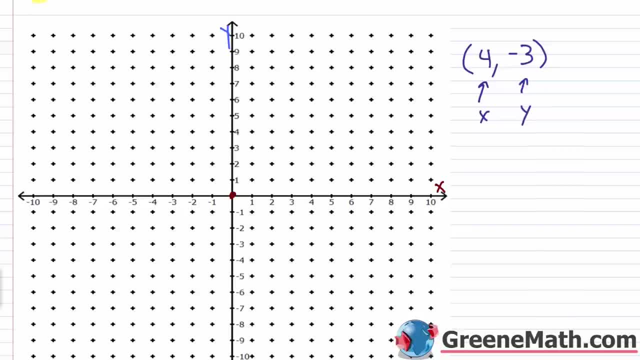 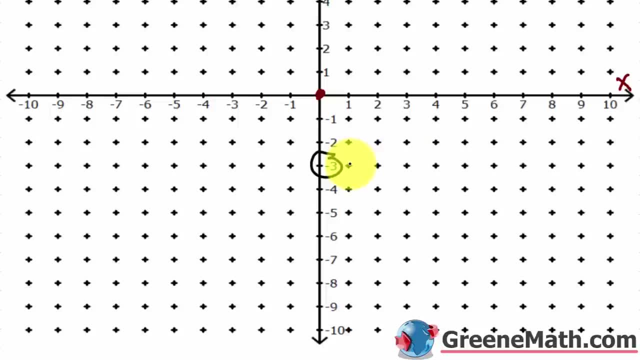 Again, this is the x value. This is the y value. So let's start out at negative three on the y axis. So let's start out here. Let's move four units to the right on the x axis. So one, two, three, four. So that's right here. And so this is going to be our point four comma negative three. Again, if I want to draw kind of some lines to show the intersection. 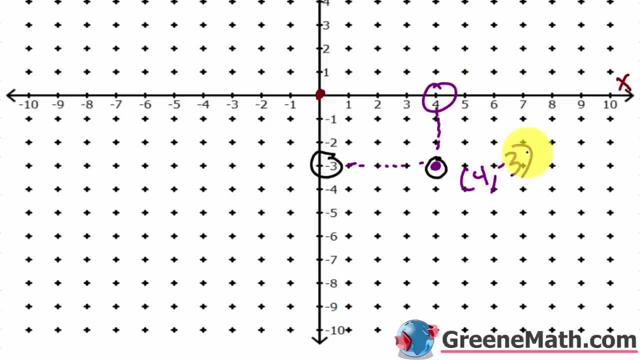 Again, this is four comma negative three. And then what quadrant does it lie in? Again, this is number one. It goes counterclockwise. 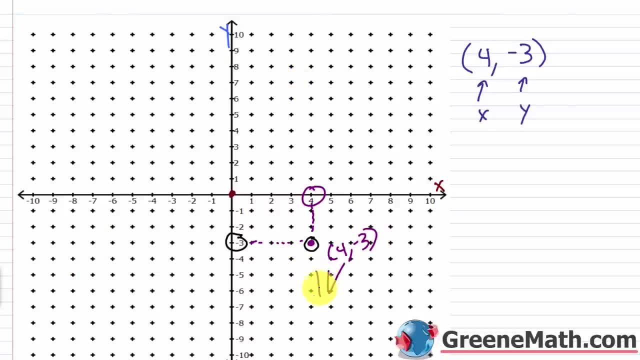 This is two, three, and then four. So it lies in the fourth quadrant. Alright, for the next one we 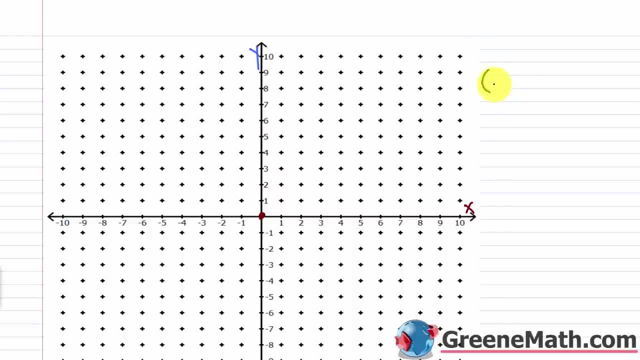 have negative nine comma negative one. So negative nine comma negative one. 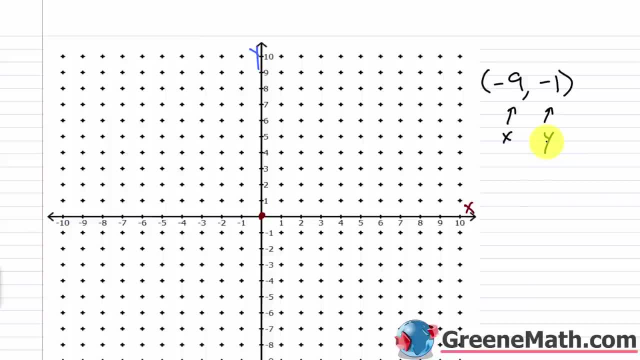 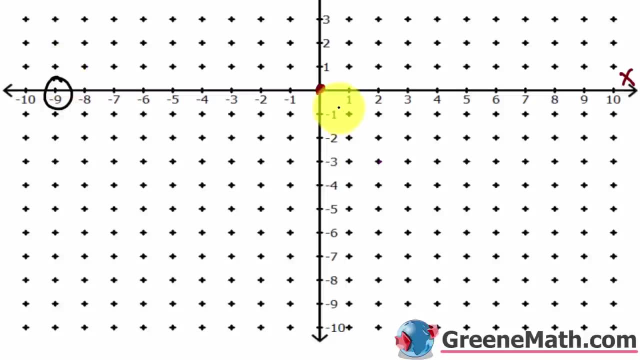 And this is your x value. This is your y value. So where is negative nine at? So negative nine on the x axis is over here. And negative one on the y axis is here. So I can go to the left nine and down one. I could go down one to the left nine. I could start out at negative nine and go down one. I could start out at negative one and go over to the left nine. 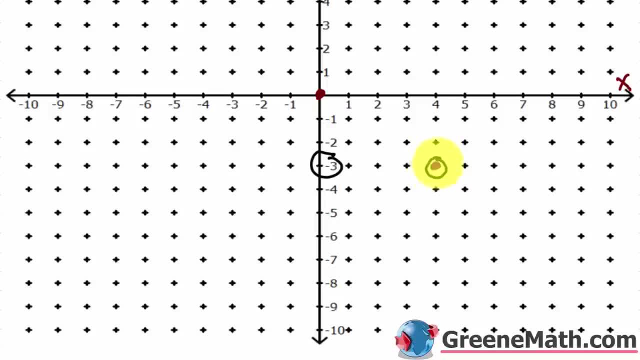 So that's right here, And so this is going to be our point: 4 comma negative 3.. Again, if I want to draw kind of some lines to show the intersection, again, this is 4 comma negative 3.. And then what quadrant does it lie in? 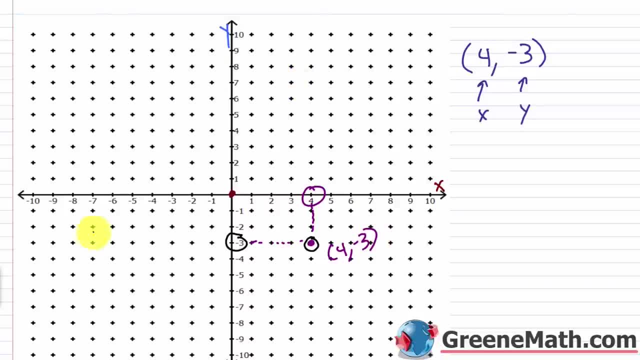 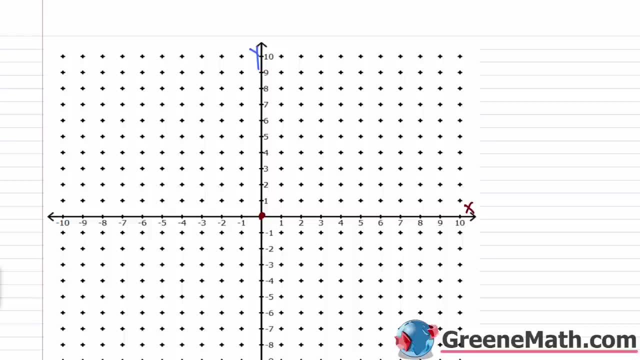 Again, this is number 1.. Goes counterclockwise: This is 2,, 3, and then 4.. So it lies in the fourth quadrant. All right, For the next one, we have negative 9 comma, negative 1.. 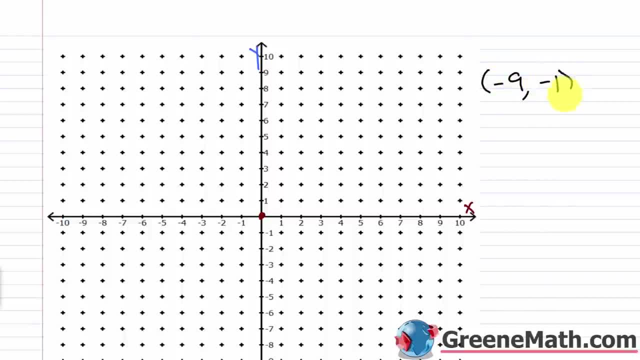 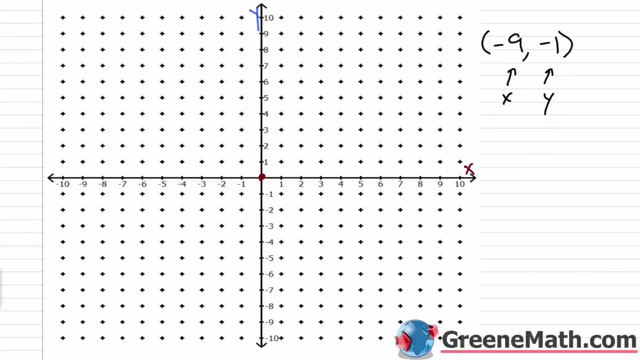 So negative 9, comma, negative 1.. And this is your x value, This is your y value. So where is negative 9 at So? negative 9 on the x axis is over here And negative 1 on the y axis is here. 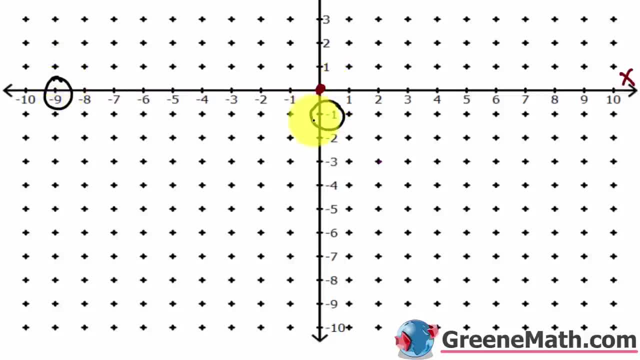 So I can go to the left 9 and down 1.. I could go down 1 to the left 9.. I could start out at negative 9 and go down 1.. I could start out at negative 1 and go over to the left 9.. 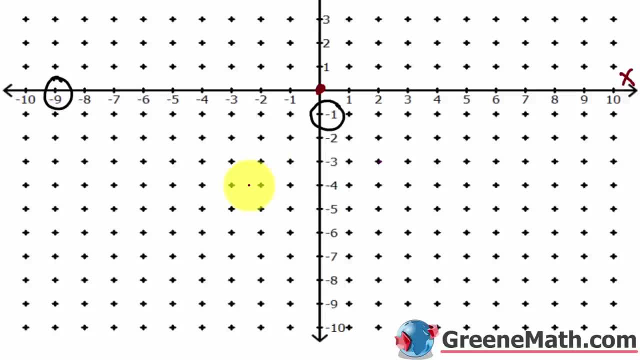 Again, it doesn't matter. Any way you kind of think about this, any way you kind of understand it, you can do it, because you're always going to end up in the same location. So this is the intersection of those two. Let me just draw that right there. 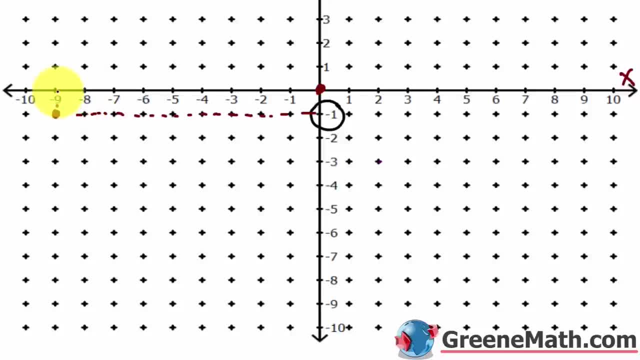 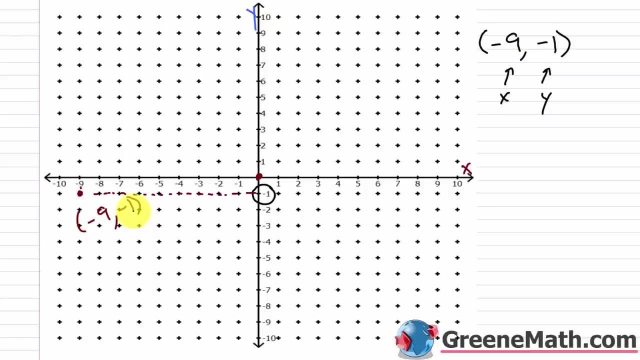 And it kind of messes up my negative 9.. So let me put this one little thing there, And I'm just going to notate that this is negative 9, comma, negative 1.. And then what quadrant does it lie in? Again, this is 1.. 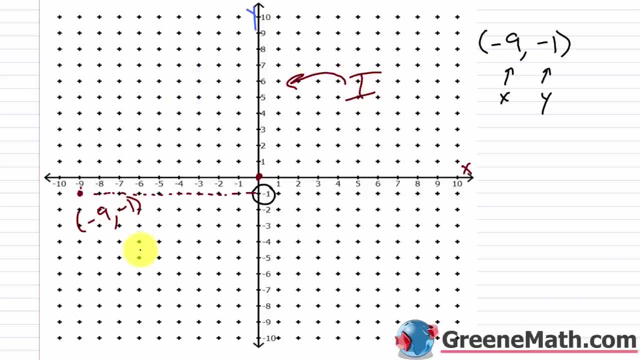 This is positive, positive, And we go this way. So this is 2.. And then this is 3.. So it lies in the third quadrant, And then this is 4.. So 2,, 3, and then 4.. 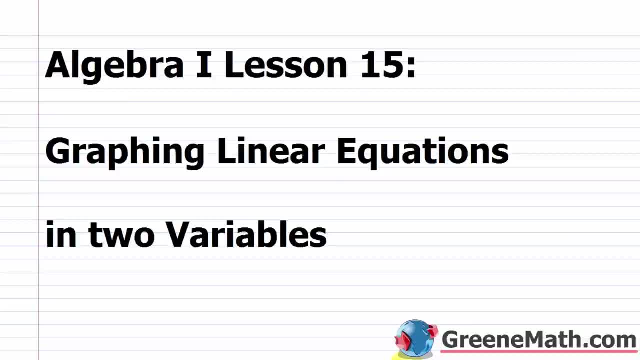 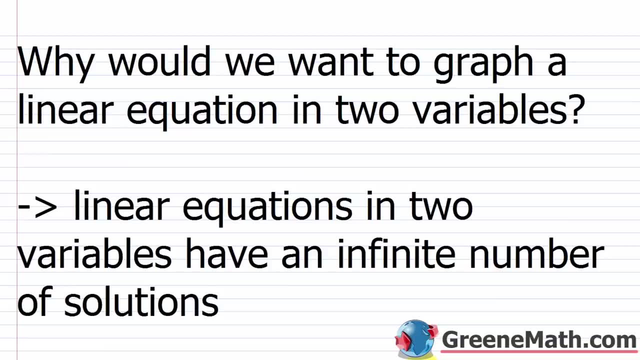 Hello and welcome to Algebra 1, Lesson 15.. In this video we're going to learn about graphing linear equations in two variables. So in the previous two lessons we developed the skills that we needed to be able to graph a linear equation in two variables. 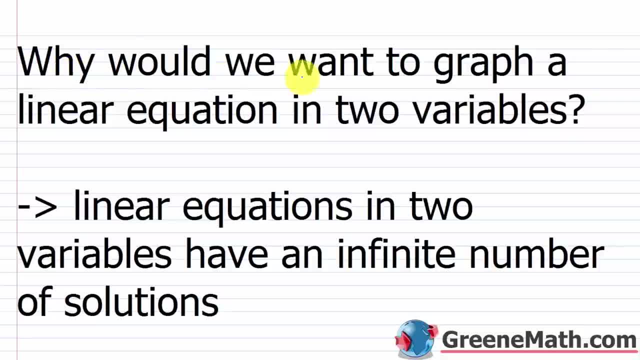 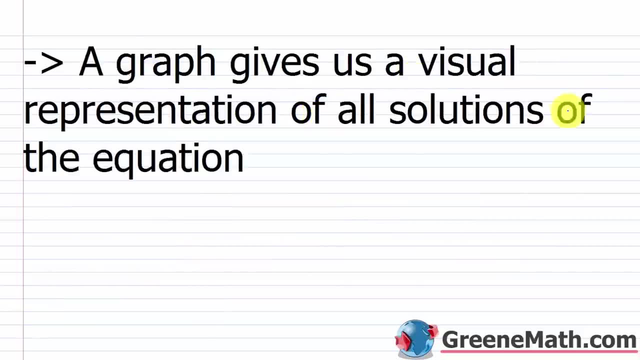 But one of the questions that might be on your mind: why would we want to graph a linear equation in two variables? Well, recall that linear equations in two variables have an infinite number of solutions. So a graph gives us a visual representation of all solutions of the equation. 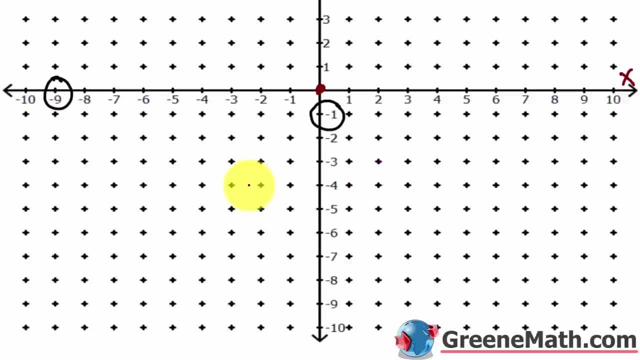 Again, it doesn't matter. Any way you kind of think about this, any way you kind of understand it, you can do it because you're always going to end up in the same location. So this is the intersection of those two. 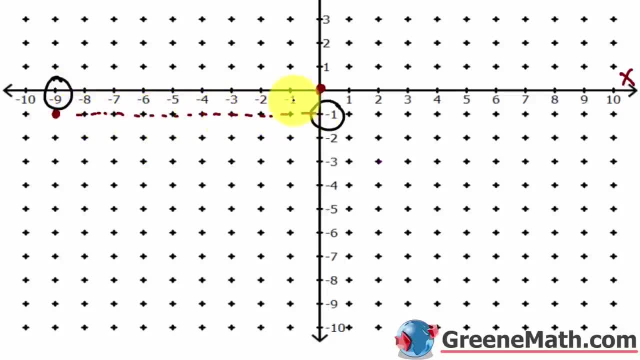 Let me just draw that right there. And it kind of messes up my negative nine. So let me put this one little thing there. And I'm just going to notate that this is 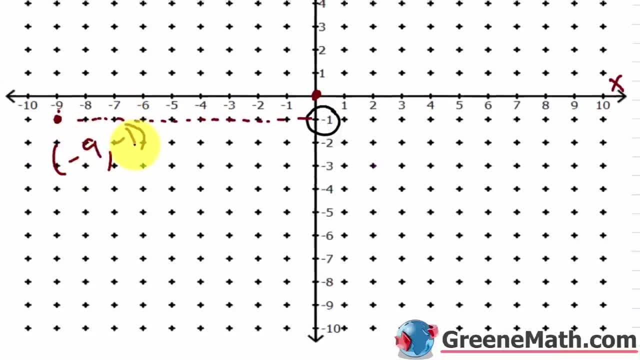 negative nine comma negative one. And then what quadrant does it lie in? Again, this is one. 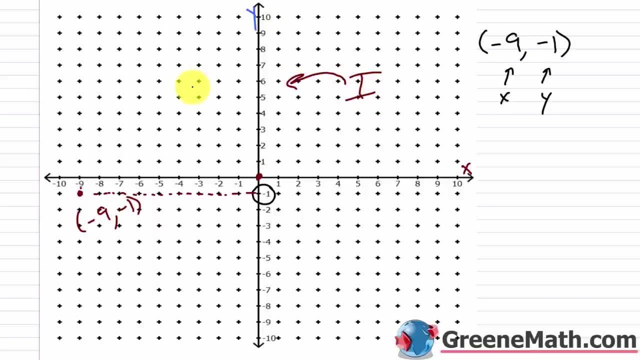 This is positive positive. And we go this way. So this is two. And then this is three. So it lies in the third quadrant. And then this is four. So two, three, and then four. 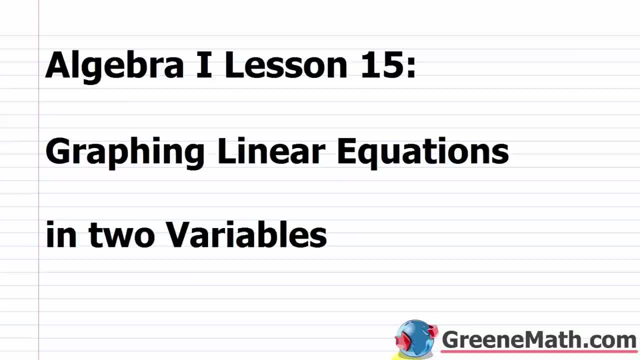 Hello and welcome to Algebra 1 Lesson 15. In this video, we're going to learn about graphing linear equations in two variables. 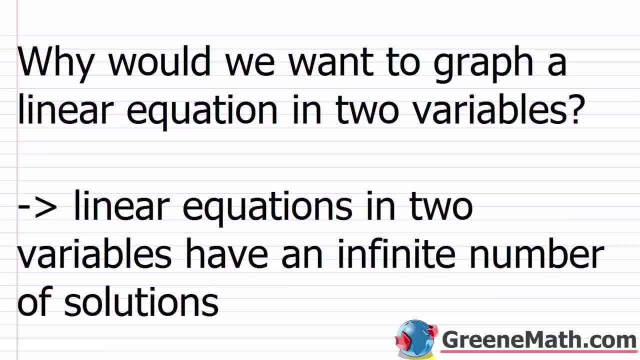 So in the previous two lessons, we developed the skills that we needed to be able to graph a linear equation in two variables. But one of the questions that might be on your mind, why would we want to graph a linear equation in two variables? Well, recall that linear equations in two variables have an infinite number of solutions. 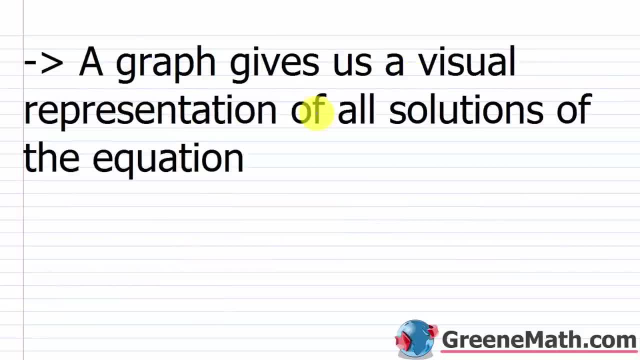 So a graph gives us a visual representation of all solutions of the equation. Now because we're graphing a linear equation in two variables, the graph is going to be a line. That's why they're called linear equations. Now each and every point on that line represents an ordered pair. 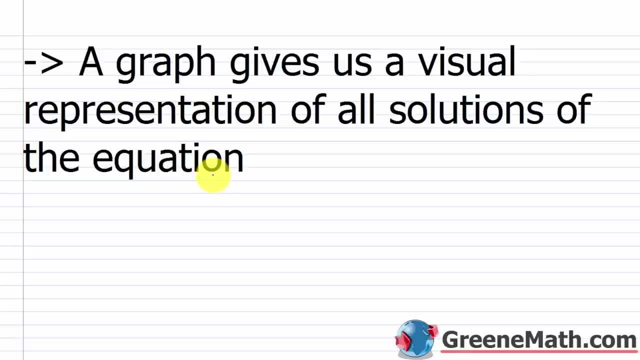 An x and a y, that is a solution for that equation. Meaning I can take the x, plug it in for x in the equation, take the y, plug it in for y in the equation, and the left and the right side will be equal. 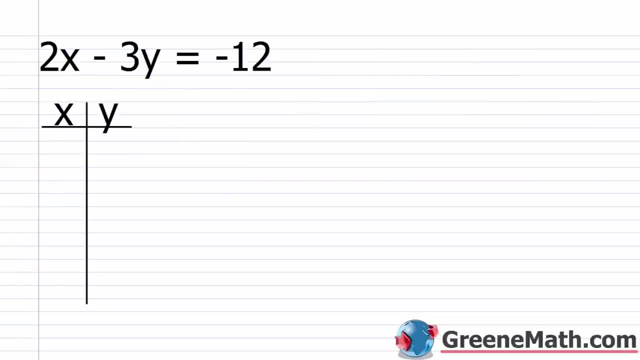 Alright, so let's get started on this topic. And it's not very difficult. 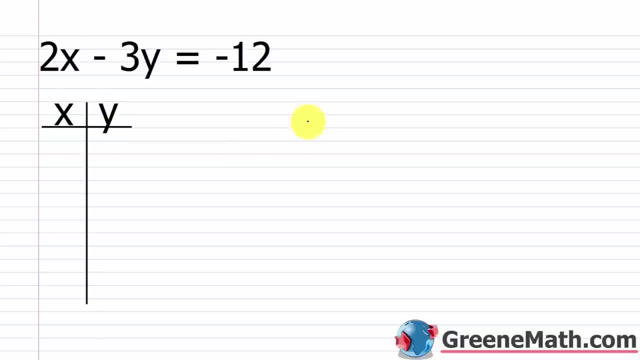 Unfortunately, the way that it's taught, in this kind of section here, you get a slow, tedious method to 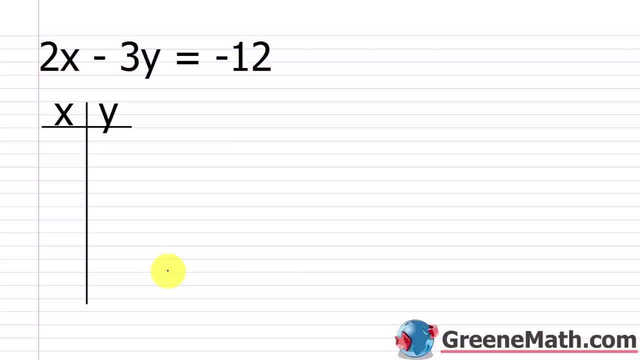 kind of execute this process. A few lessons from now, when we start talking about slope, when we start talking about 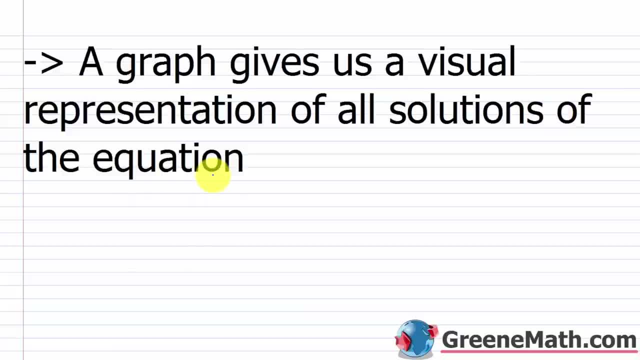 Now, because we're graphing a linear equation in two variables, the graph is going to be a line. That's why they're called linear equations. Now, each and every point on that line represents an ordered pair: An x and a y. That is a solution. 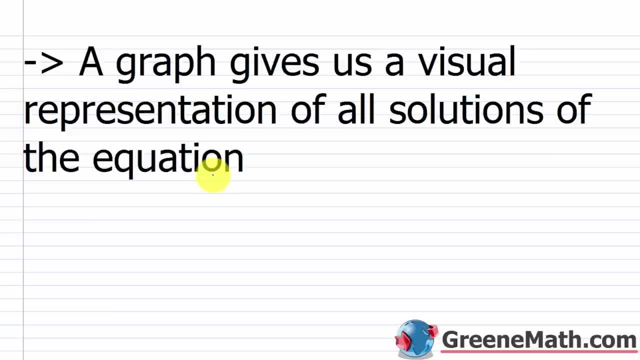 So a graph is a linear equation. So I can take the x and plug it in for x in the equation, Take the y and plug it in for y in the equation, And the left and the right side will be equal. Alright, so let's get started on this topic. 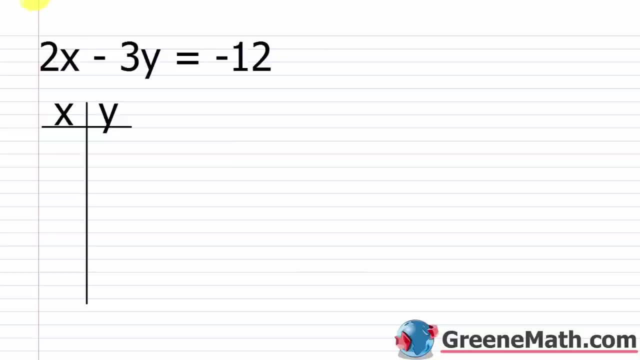 It's not very difficult. Unfortunately, the way that it's taught in this kind of section. here you get a slow, tedious method to execute this process. A few lessons from now, when we start talking about slope, When we start talking about solving. 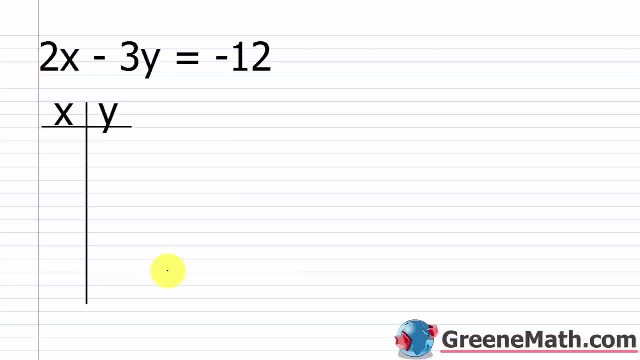 And I just want to say this: for y and all these other things, you're going to get a much faster way to graph a linear equation of two variables. in fact, if you solve the equation for y, it's very, very, very quick. but for right now, 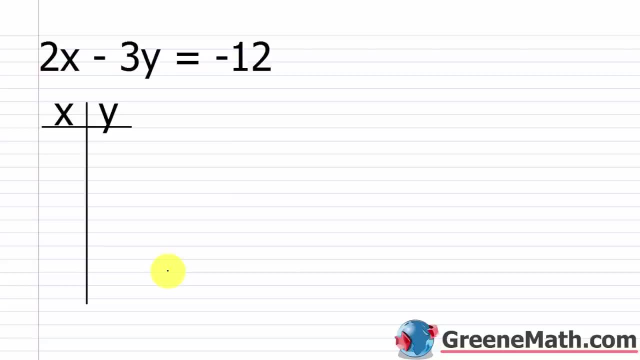 we're going to kind of start out slow and i'm going to teach you this method that uses a table of values. so we have our equation: 2x minus 3y equals negative 12, and i have a table right here with x and with y. so in a previous lesson i gave you an x value and you solved for y. 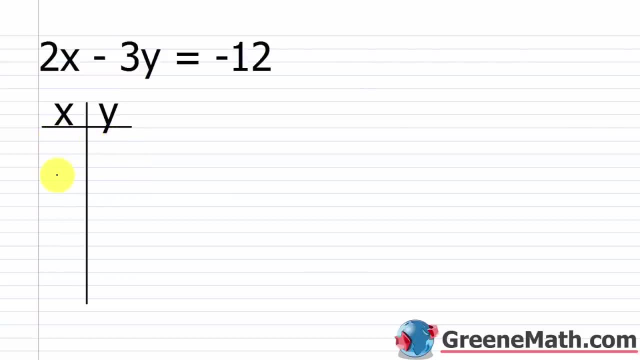 or i gave you a y value and you solved for x. here you can come up with whatever x and solve for y, or come up with whatever y and solve for x that you want. keep in mind that you have to plot these on a coordinate plane, so you want to keep them nice and small and you want to work with integers if 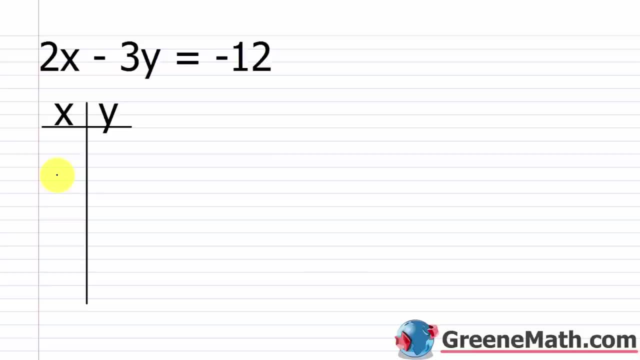 possible because your scale on the coordinate plane is generally going to be in integers. so let's go ahead and start out by picking a value for x so you can choose numbers at random. but you're going to see later on that it usually works best to work with the number zero. so let's plug in. 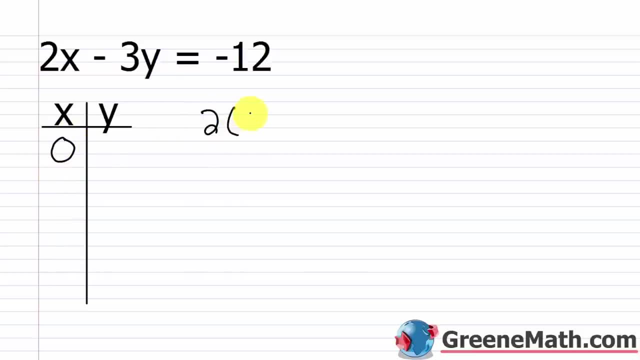 a zero for x and i would have: 2 times 0 minus 3y equals negative 12. so if x is zero, what's y going to be? well, this is going to go away. 2 times 0 is 0 and i'll have negative 3y equals negative 12. 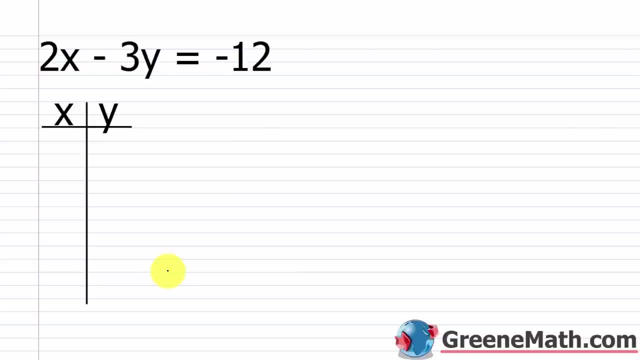 solving for y and all these other things, you're going to get a much faster way to graph a linear equation in two variables. In fact, if you solve the equation for y, it's very, very, very quick. 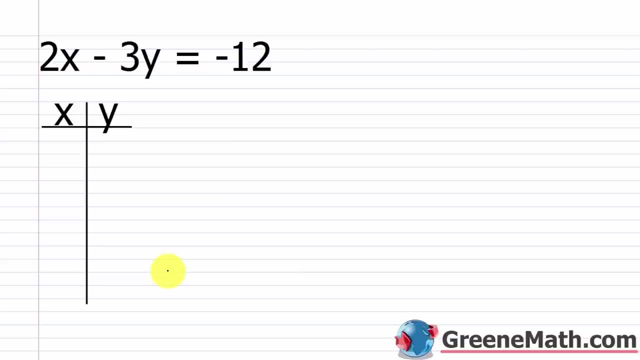 But for right now, we're going to kind of start out slow, and I'm going to teach you this method that uses a table of values. So we have our equation 2x minus 3y equals negative 12. And I have a table right here with x and with y. So in a previous lesson, I gave you an x value, and you solved for y. 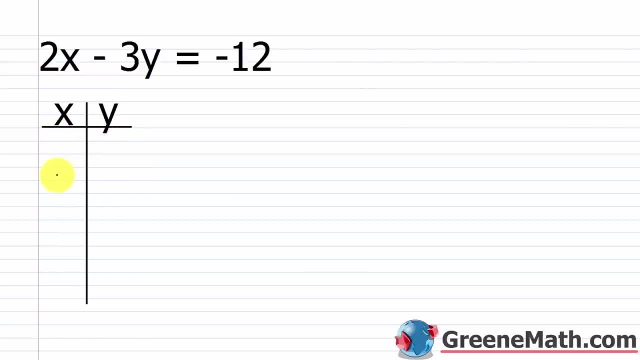 Or I gave you a y value, and you solved for x. Here, you can come up with whatever x and solve for y, or come up with whatever y and solve for x that you want. Keep in mind that you have to plot these on a coordinate plane. So you want to keep them nice and small, and you want to work with integers if possible because your scale on the coordinate plane is generally going to be in integers. 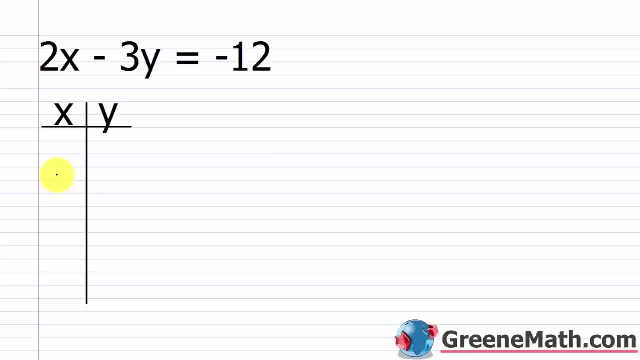 So let's go ahead and start out by picking a value for x. So you can choose numbers at random, but you're going to see later on that it usually works best to work with the number 0. So let's plug in a 0 for x, and I would have 2 times 0 minus 3y equals negative 12. So if x is 0, 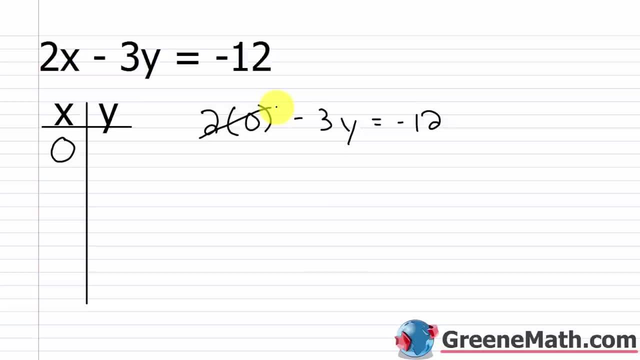 what's y going to be? Well this is going to go away. 2 times 0 is 0. 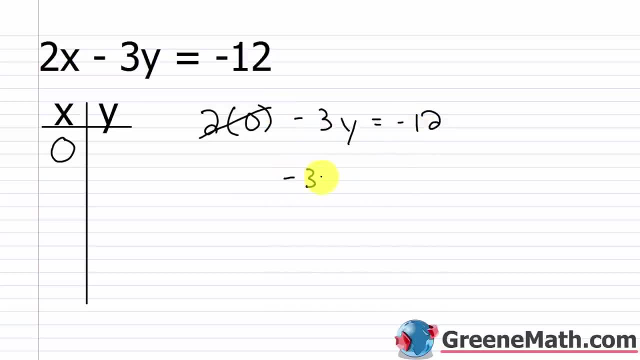 And I'll have negative 3y equals negative 12. 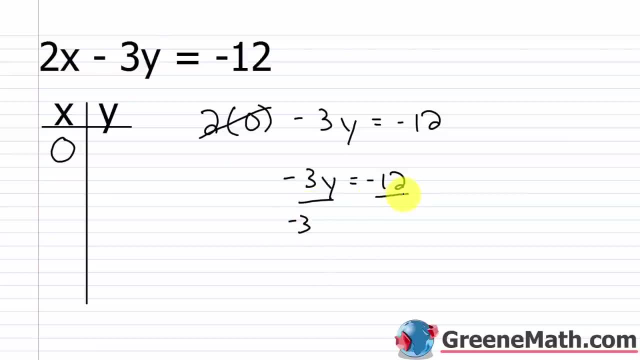 Divide both sides of the equation by negative 3. 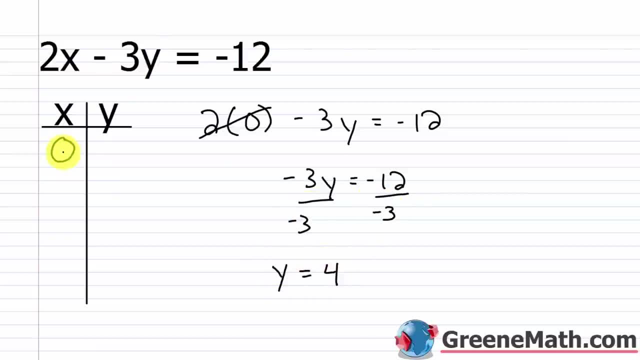 And I'll get y is equal to 4. So if x is 0, y is 4. 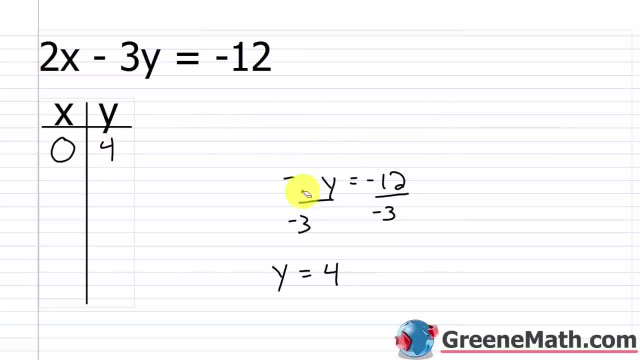 So that's one ordered pair that we would have. Now how many do we need? Well you're going to find out in your textbook, or from somebody, 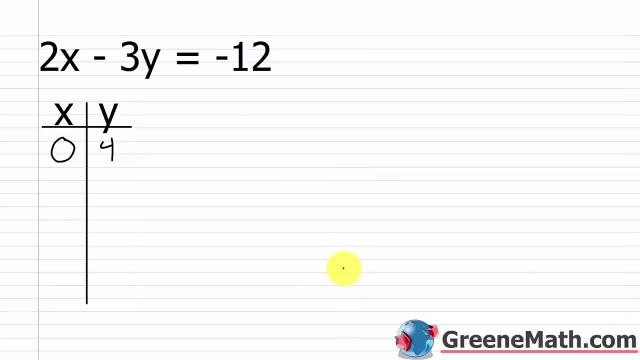 that two ordered pairs are two points as we call them, make a line. 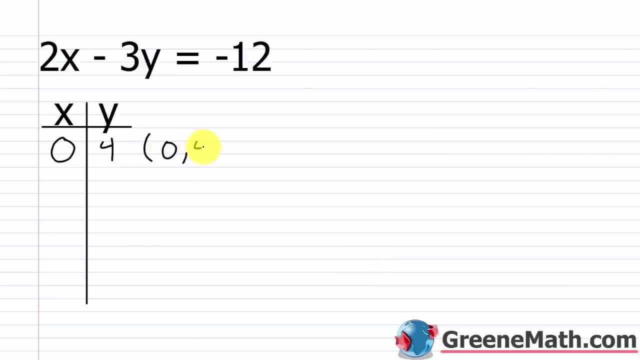 But, when you're doing this, you want to always use 3, because the third point is going to check to make sure that you have a line. 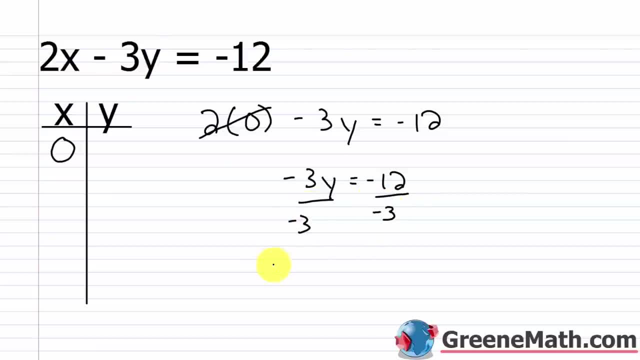 divide both sides of the equation by negative 3 and i'll get: y is equal to 4. so if x is 0, y is 4. so that's one ordered pair that we would have. now how many do we need? well, you're going to find out. 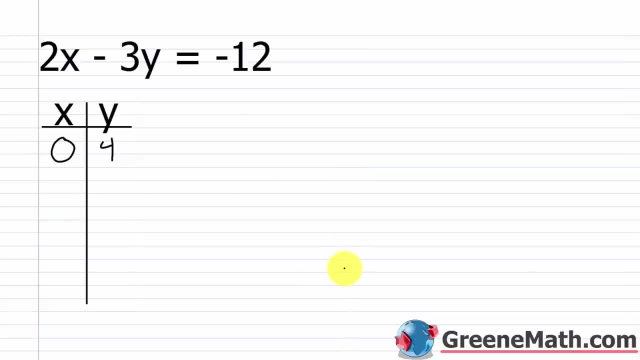 in your textbook or from somebody, that two ordered pairs, or two points as we call them, make a line. but when you're doing this, you want to always use three, because the third point is going to check to make sure that you have a line. so, in other words, if i get a point here and my, your Chance. lose, i'll have to check somewhere else. it could wind up having a dimensional marker and you'll get an English number that's going to get the number three wrong, unless i write negative to my equation there, because my equation could change that. so I don't want to theirs because I don't want to. 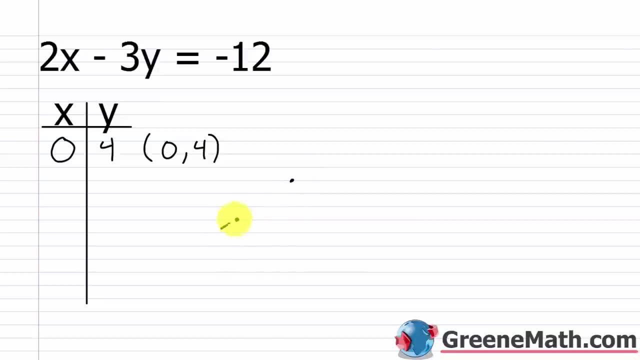 so if I get a four, to keep both sides. I don't want negative three soient to measure positive. if I get a point here and let's say here, yeah, I can draw a line connecting those points, but let's say a third point would have been down here, well, that's not a line. I must have made a mistake if. 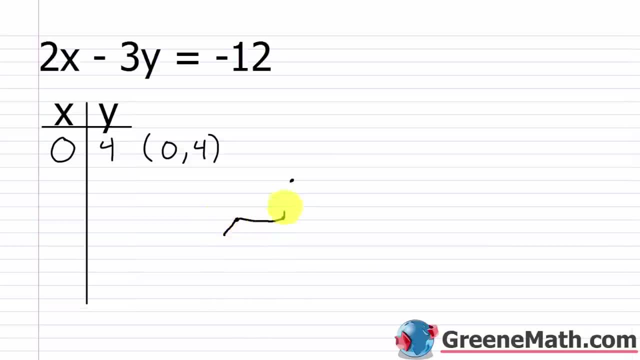 I'm trying to draw a graph there. it'd be something like this: right, I mean, that's, that's not a line. so if you get a third point that's not in line, meaning it doesn't look like this, let's say this point was right here. then you know, you're okay. so that's why that third point is used as. 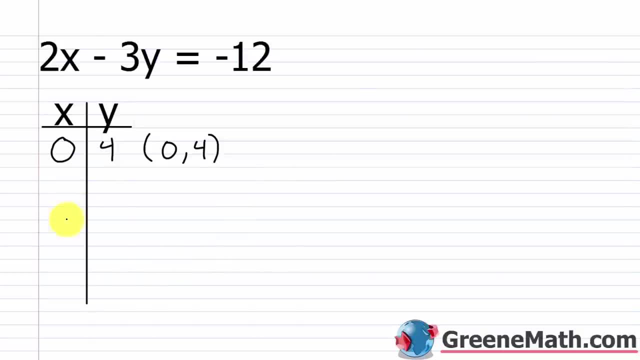 a check. so now I'm going to get two additional points again. keep in mind, you want to choose some nice small integer values, so I'm going to choose something. for x, let's say I choose the number one. so 2 times 1 minus 3y equals negative 12. 2 times 1 is 2, so we get 2 minus 3y equals. 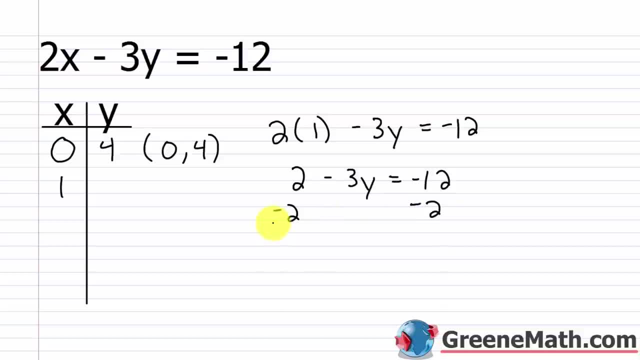 negative 12. subtract 2 away from each side of the equation, I'd have negative 3y is equal to negative 14. divide both sides equation by negative 3 and I'm going to get that y is equal to 14 thirds. now if I'm using a computer or something, I can plot the point 1 comma, 14 thirds. 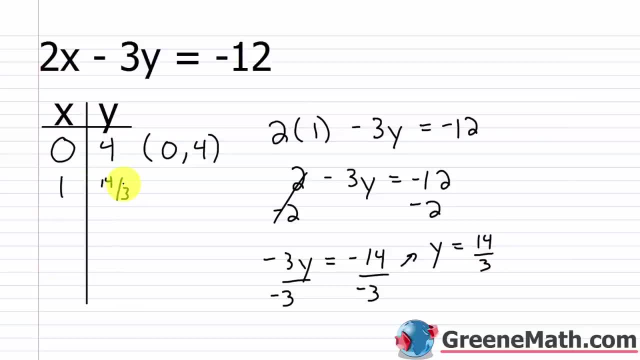 but if I'm doing this on paper, do I really want to work with something like that? no, so if I get a non-integer value, I just kind of move on and try something else. I don't want to work with that because it's too hard to plot it on the corner. 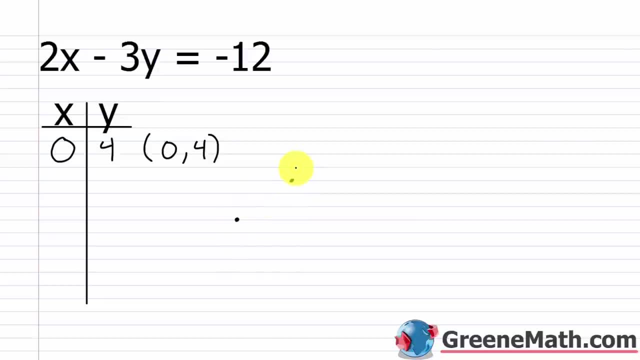 So in other words, if I get a point here, and let's say here, yeah I can draw a line connecting those points, but let's say a third point would have been down here. Well that's not a line. I must have made a mistake. If I'm trying to draw a graph there, it'd be something like this, right? I mean that's not a line. So if you get a third point that's not in line, meaning it doesn't look like this, let's say this point was right here, then you know you're okay. So that's why that third point is used as a check. 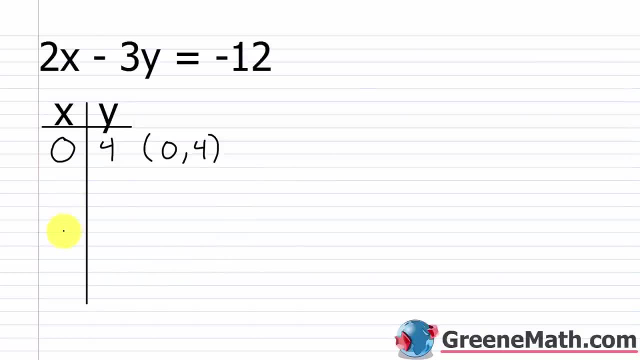 So now, I'm going to get two additional points. Again, keep in mind you want to choose some nice small integer values. So I'm going to choose something for x. Let's say I choose the number 1. So 2 times 1 minus 3y equals negative 12. 2 times 1 is 2, so we get 2 minus 3y equals negative 12. 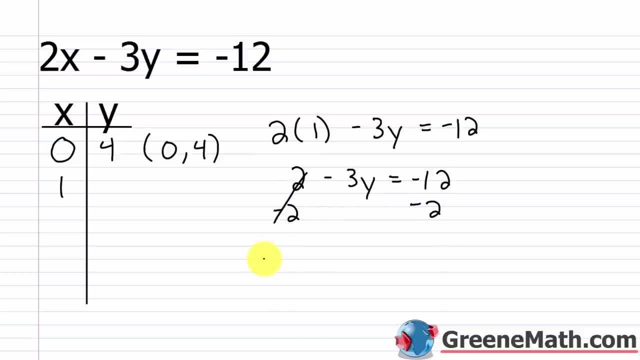 Subtract 2 away from each side of the equation. I'd have negative 3y is equal to negative 14. 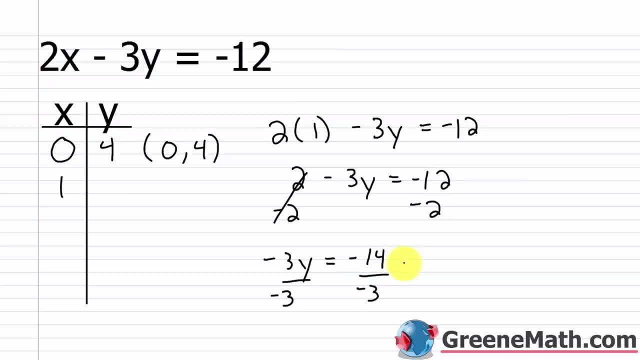 Divide both sides of the equation by negative 3. And I'm going to get that y is equal to 14 thirds. 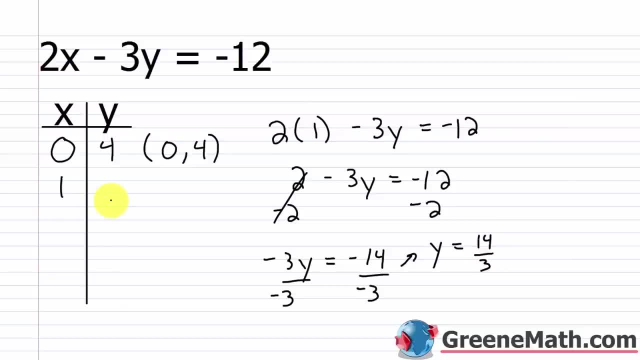 Now if I'm using a computer or something, I can plot the point 1 comma 14 thirds. 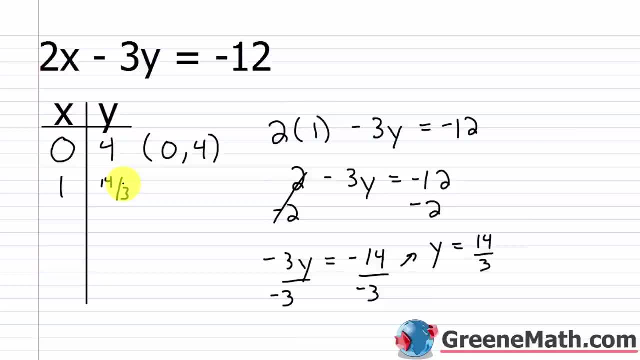 But if I'm doing this on paper, do I really want to work with something like that? No. So if I get a non integer value, I just kind of move on and try something else. I don't want to work with that because it's too hard to plot it 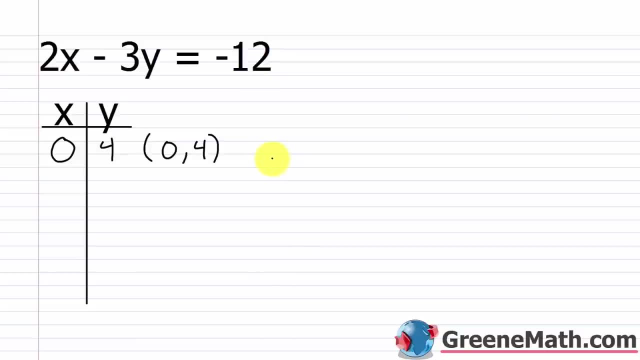 on the coordinate plane. So let's think about something for a second before we move on. We have 2x minus 3y equals negative 12. 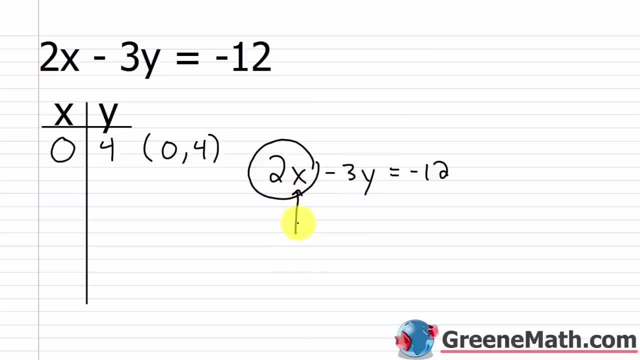 If I think about this right here, whatever I plug in for x, I'm going to multiply it by 2. Then I'm going to subtract away, or add, depending on whether it's positive or negative, to both sides of the equation. So that's going to end up being over here. Whatever value that is over here, it's got to be divisible by negative 3, otherwise it's not going to be an integer. 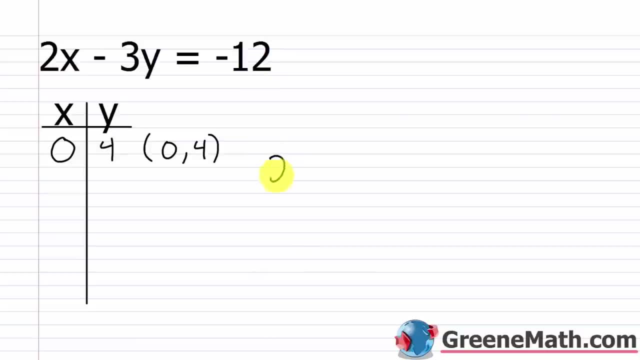 plane. so let's think about something for a second before we move on. we have 2x minus 3y equals negative 12. if I think about this right here, whatever I plug in for x, I'm going to multiply it by 2, then I'm going to subtract away or add, depending on whether it's positive or negative. 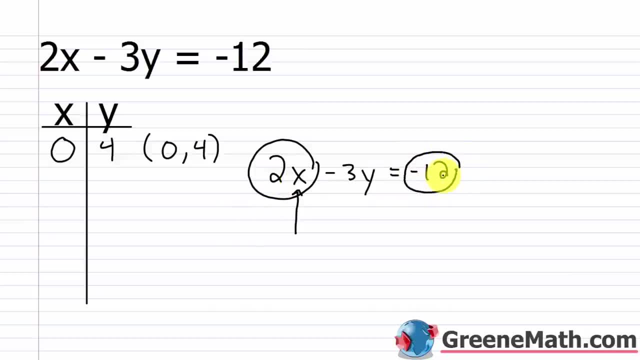 to both sides of the equation. so that's going to end up being over here. whatever value that is over here, it's got to be divisible by negative 3, otherwise it's not going to be an integer. so keep that in mind. so one thing I can do is I can say: okay if I plug in a 3 here. I know that 2 times 3 is 6, so 2 times 3 is 6. 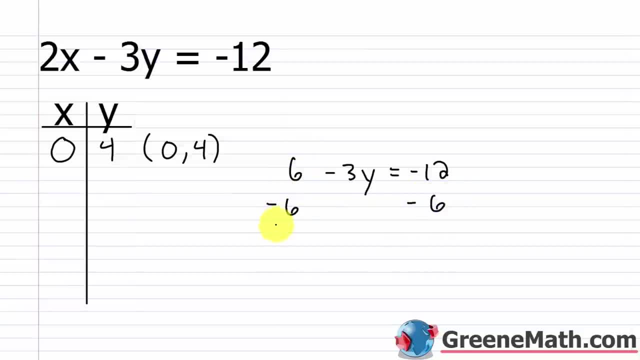 and if I subtract 6 away from each side of the equation that's gone, I'll have negative 3y is equal to negative 18. well, negative 18 is divisible by negative 3. so if x is 3- remember I plugged in a 3 for x- y would be divide both sides by negative 3 and I would get y equals positive 6. so there's an. 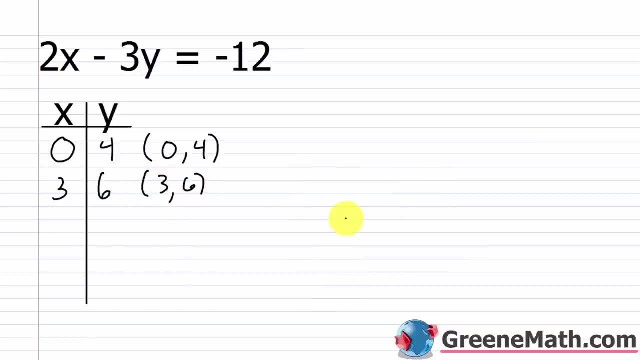 expression over here: 2 times 2 is minus cos 3, then negative 4ומa 3 is minus 1 above 5b. now I put in this plus 2 Rashlings and I could do this with negative 2, and I could also do this with negative 3, so 2 times negative 3 Minister. 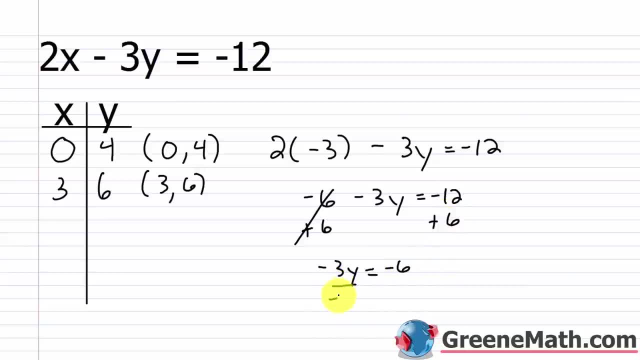 no 3 is negative. 6 minus 3 y equals negative 12. I would add 6 to both sides of the equation. that's gone. I'd have negative 3. y is equal to negative 12 plus 6 is negative 6. divide both sides. 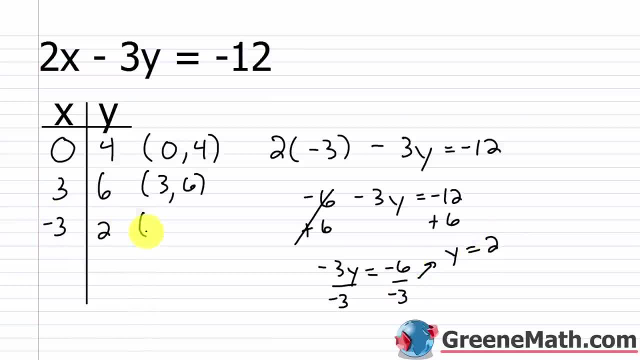 by negative 3, 3, y is 2.. All right, so now, once I've done that kind of scratch paperwork, I'm ready to move on and actually graph my equation. So how do I do that? Well, I said that I needed three, ordered 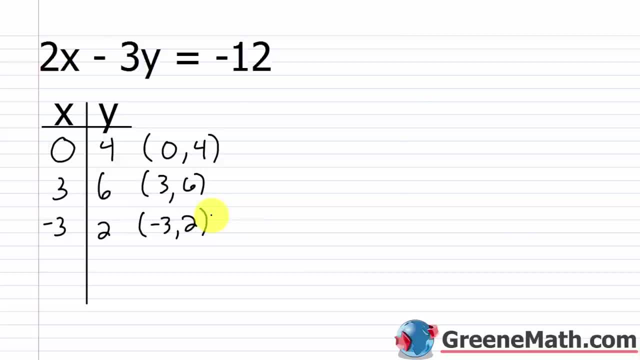 pairs- really two make a line, but the third is for the check, And so I take my ordered pairs down to the coordinate plane and I plot them, just like I did in the last lesson, only now I'm going to draw a straight line through them. when I'm done, Let's take this down to the coordinate plane. 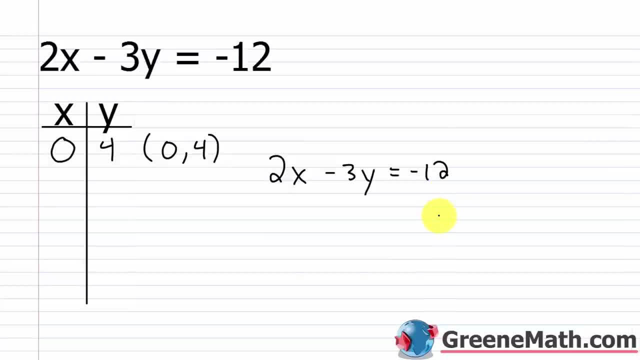 So keep that in mind. So one thing I can do is I can say okay, if I plug in a 3 here, I know that 2 times 3 is 6. So 2 times 3 is 6. And if I subtract 6 away from each side of the equation, that's gone. I'll have negative 3y is equal to negative 18. Well negative 18 is divisible by negative 3. So if x is 3, remember I plugged in a 3 for x, y would be divide both sides by negative 3, and I would get y equals 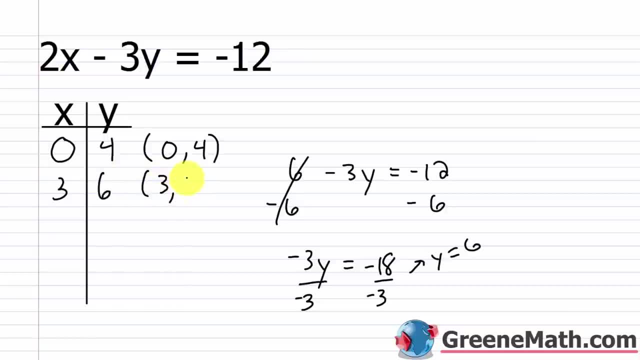 positive 6. So there's an ordered pair. 3 comma 6. And I could also do this with negative 3. So 2 times negative 3 minus 3y equals negative 12. 2 times negative 3 is negative 6. Minus 3y equals negative 12. I would add 6 to both sides of the equation. That's gone. 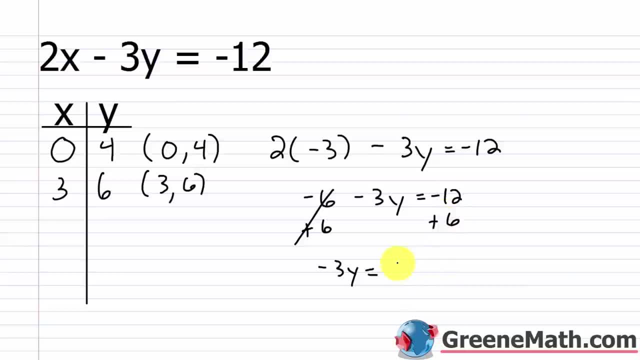 I'd have negative 3y is equal to negative 12 plus 6 is negative 6. Divide both sides by negative 3, and you're going to get that y is equal to negative 6 over negative 3 is 2. So if x is negative 3, y is 2. 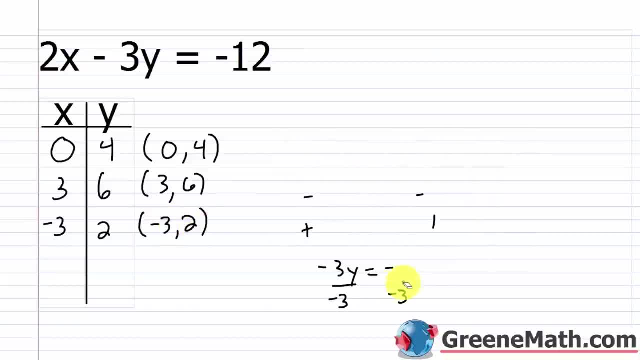 Alright, so now once I've done that kind of scratch paper work, I'm ready to move on and actually graph my equation. 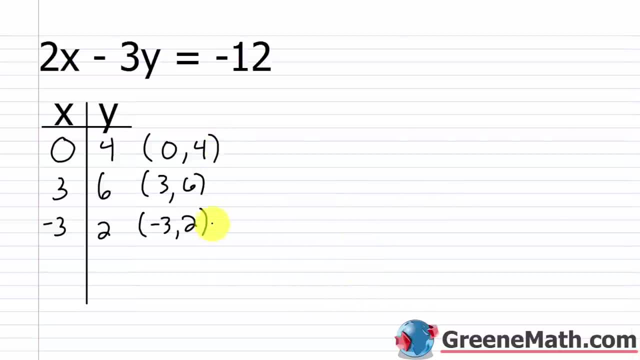 So how do I do that? Well I said that I needed 3 ordered pairs, really 2 make a line, but the third is for the check. And so I take my order pairs down to the coordinate plane, and I plot them, just like I did in the last lesson, only now I'm going to draw a straight line through them when I'm done. Let's take this down to the 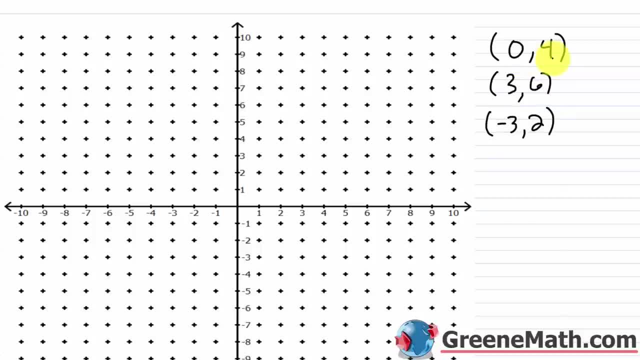 coordinate plane. Alright, so we have the ordered pair . 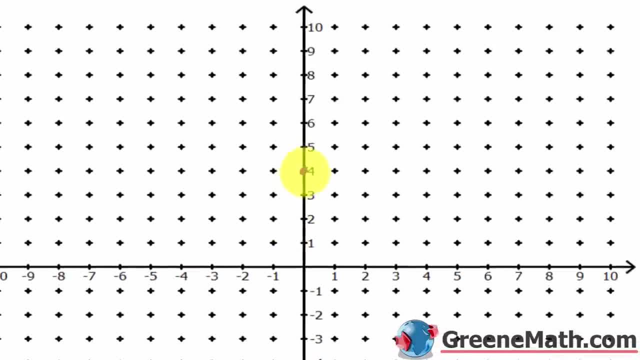 So let's plot that. So is right here. Then we have the ordered pair . 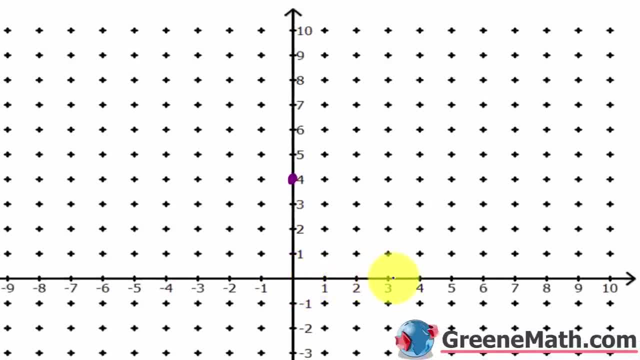 So I want to go 3 units to the right, and 6 units up. That's going to be right here. I'm going to have the ordered pair . 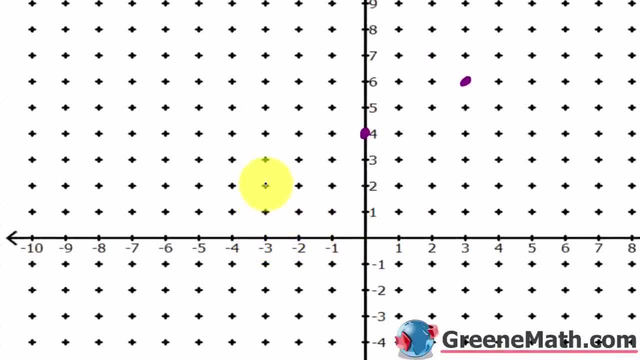 So I'm going to go 3 units to the left, and 2 units up. 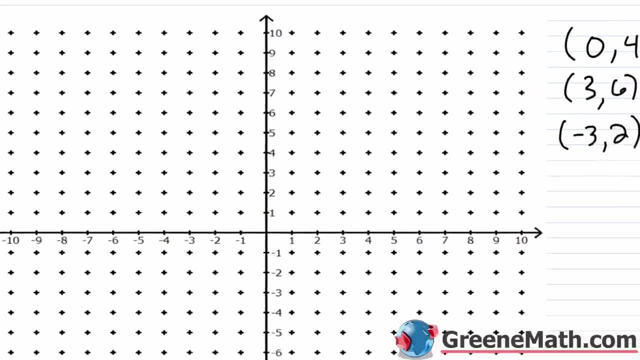 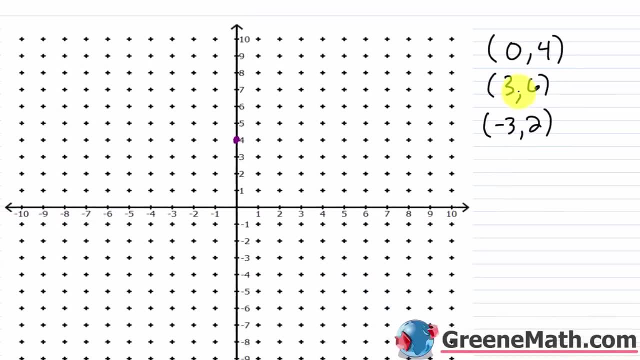 All right. so we have the ordered pair 0, 4.. So let's plot that. So 0, 4 is right here. Then we have the ordered pair 3, 6.. So I want to go three units to the right and six units up. 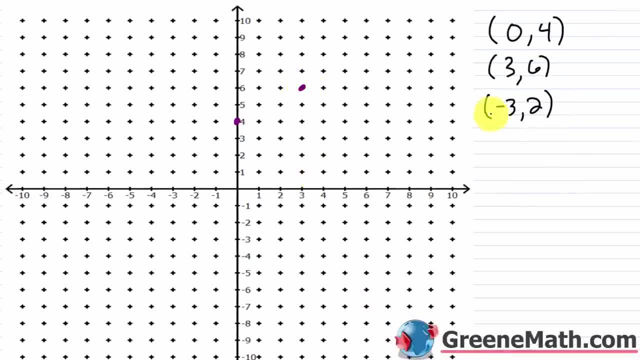 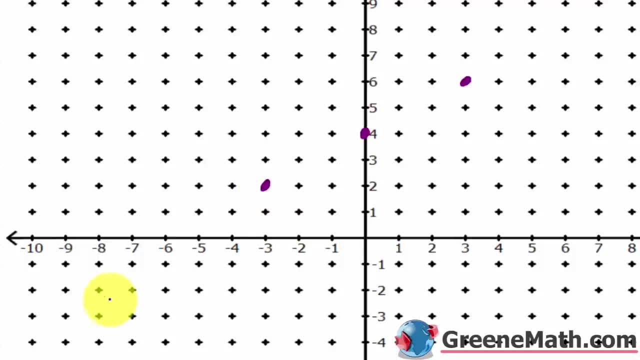 That's going to be right here. Then I have the ordered pair negative 3, 2.. So I'm going to go three units to the left and two units up And you can eyeball that and see that you could draw a straight line through that. 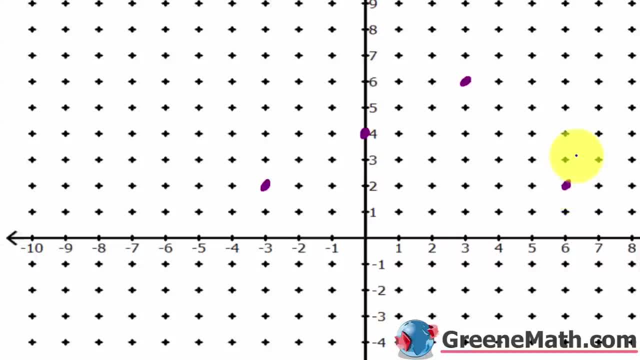 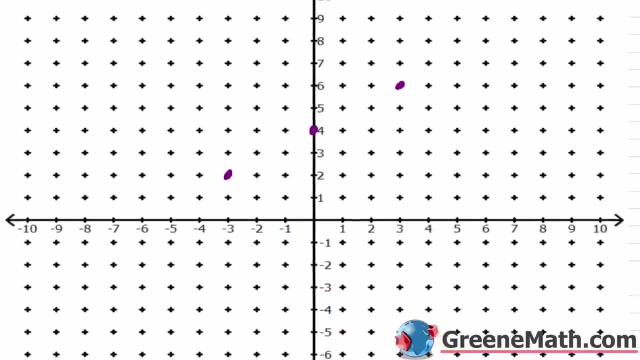 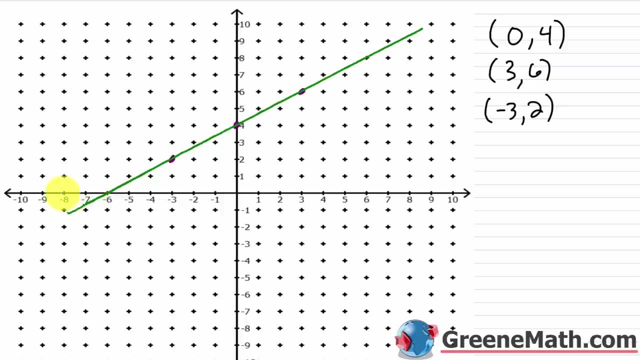 If one of your points was somewhere way over here, you have a problem. You need to go back and look at it and check your math. You did something wrong, Okay, so now all I want to do is draw a line through the points. Now, in most cases, you're not going to be able to draw. 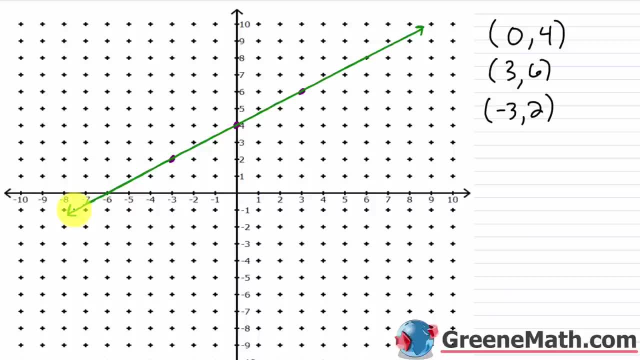 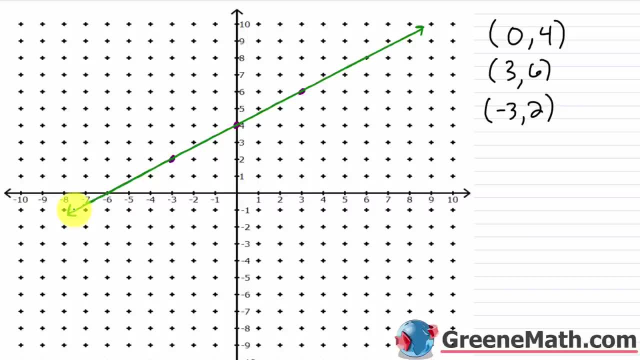 just a piece of loose leaf and no ruler. So just do the best you can Make it obvious to the teacher that you know you gave an effort to draw a straight line through the points And in most cases they're going to be nice and give you credit. But unless you're using a computer, 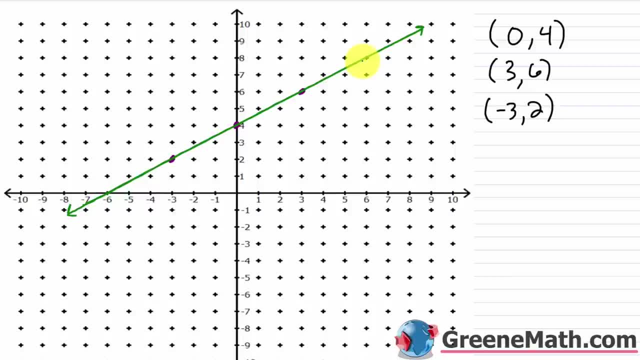 it's almost impossible to draw a completely perfect line. So then, one of the things you can do: when you're done, you can label it. So this is the graph of the equation: 2x minus 3y is equal to negative 12.. And notice that each and every point on that line, again, is an ordered. 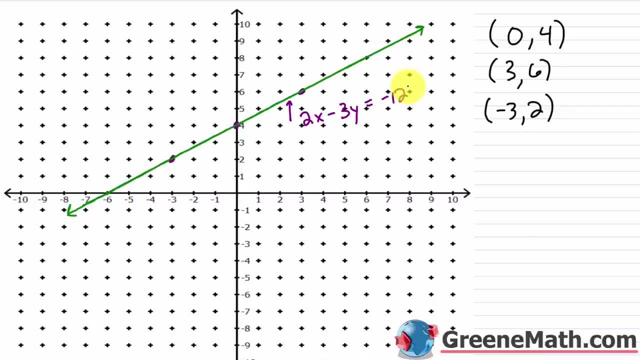 pair, that is a solution to the equation. So, for example, it looks like this point right here is on the line. Hopefully I drew it straight enough to where it is, So that would be the point 6, 8.. So 6, 8.. Let's see if that works as a solution. 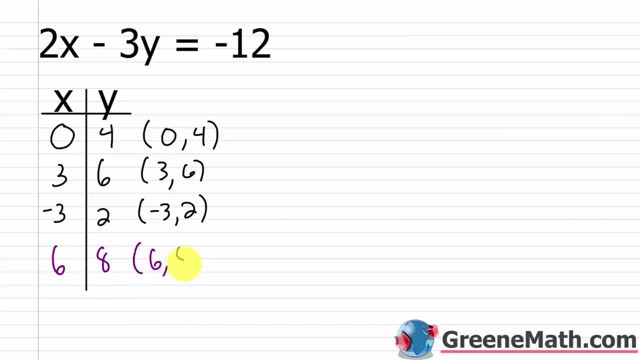 So let's test an x value of 6, a y value of 8.. Let's see if that works. So 2 times 6 minus 3 times 8 should be equal to negative 12.. 2 times 6 is 12 minus 3 times 8. That's 24 equals negative. 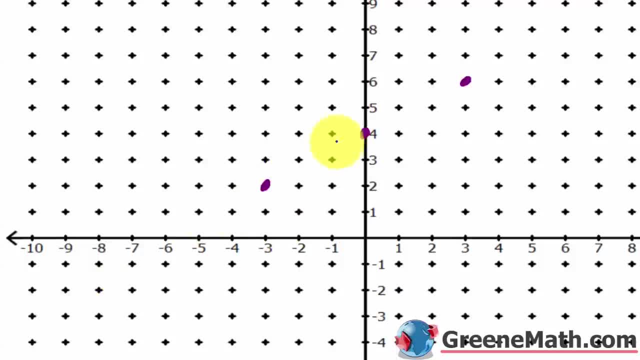 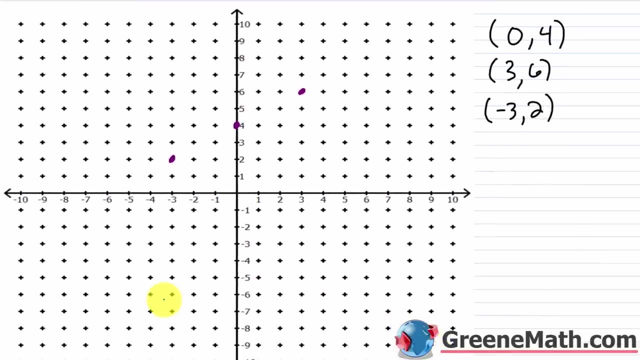 And you can eyeball that and see that you can draw a straight line through that. If one of your points was somewhere way over here, you have a problem. You need to go back and look at it and check your math. You did something wrong. Okay, so now all I want to do is draw a line through the points. 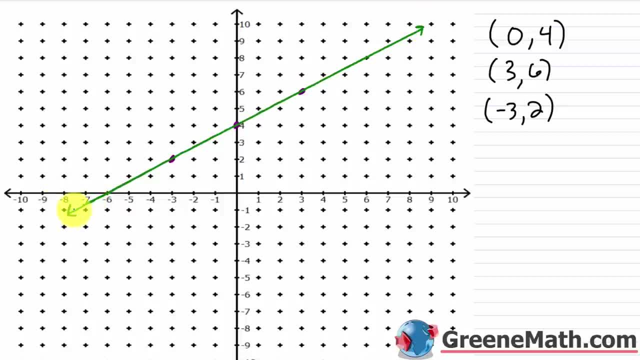 Now, in most cases, you're not going to be able to draw a perfect line. You've got a ruler at best, and you've got a piece of graph paper, hopefully. But some of us are going to be using just a piece of loose leaf and no ruler. So just do the best you can. Make it obvious to the teacher that you gave an effort to draw a straight line through the points. 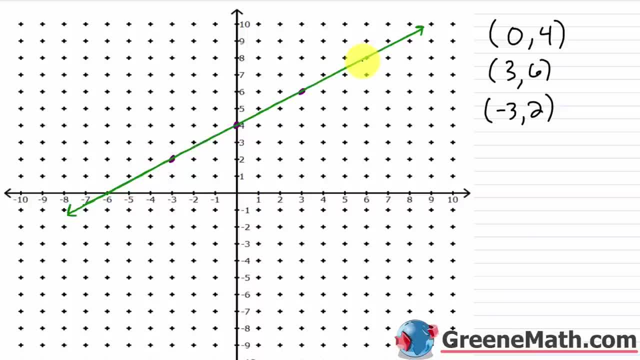 And in most cases, they're going to be nice and give you credit. But unless you're using a computer, it's almost impossible to draw a completely perfect line. 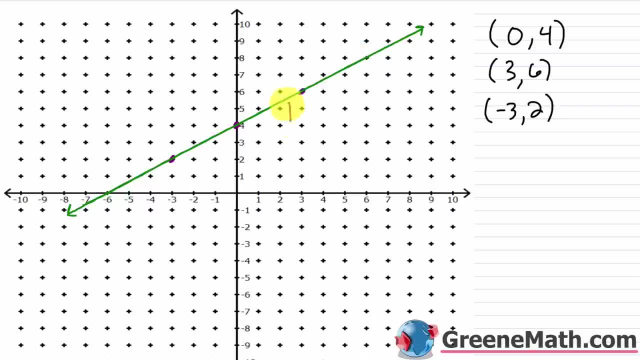 So then one of the things you can do when you're done you can label it. So this is the graph of the equation 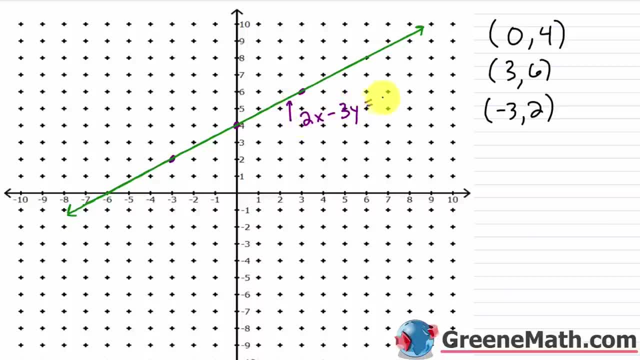 2x minus 3y is equal to negative 12. And notice that each and every point on that line, again, is an ordered pair that is a solution to the equation. 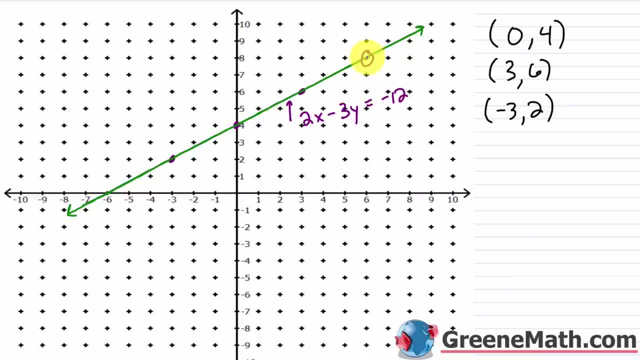 So for example, it looks like this point right here is on the line. Hopefully I drew it straight enough to where it is. So that would be the point . So . Let's see if that works as a solution. So let's guess an x value of 6, a y value of 8. Let's see if that works. 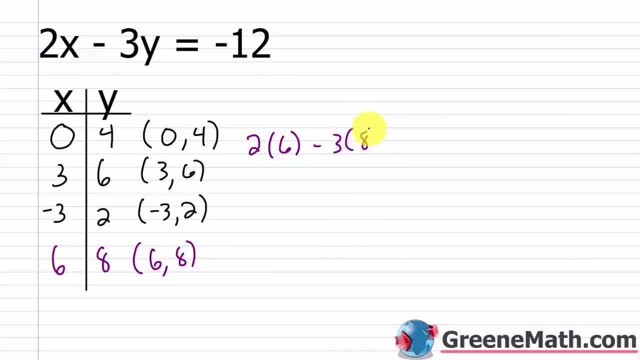 So 2 times 6 minus 3 times 8 should be equal to negative 12. 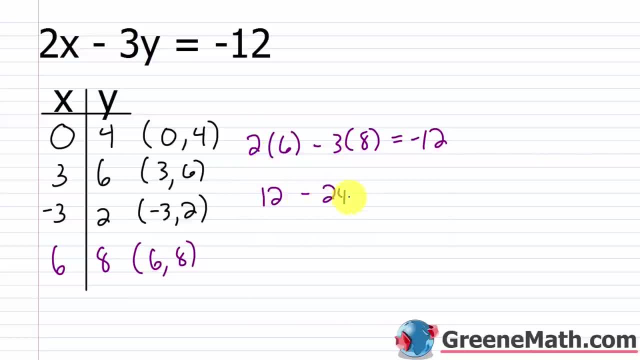 2 times 6 is 12. Minus 3 times 8, that's 24, equals negative 12. You can see that works out. 12 minus 24 is negative 12. 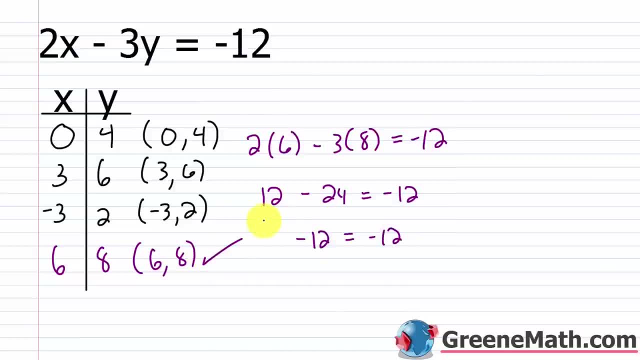 So you get negative 12 equals negative 12. So yeah, that's a solution to 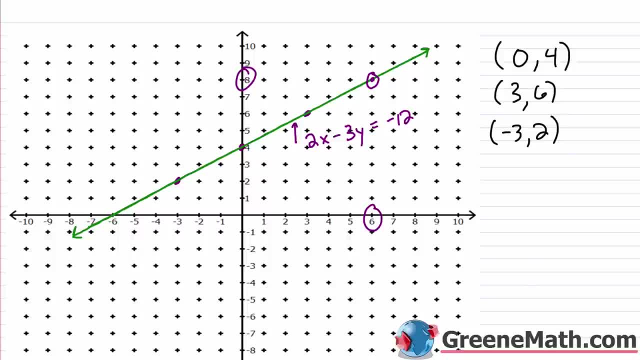 the equation. So that's the general idea behind graphing a linear equation into variables. 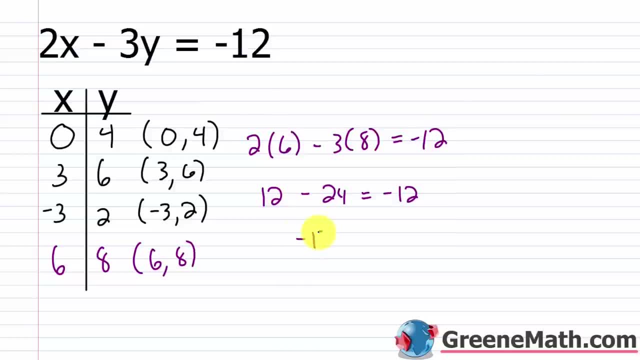 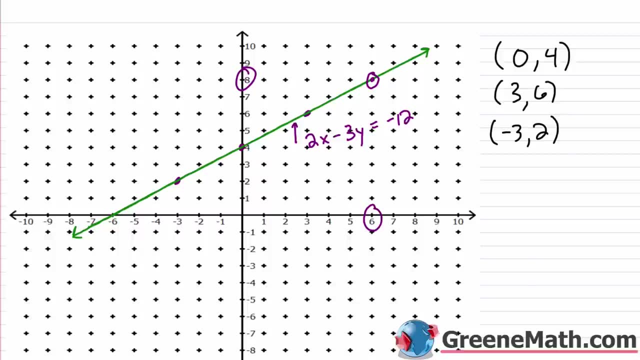 12.. You can see that works out: 12 minus 24 is negative 12.. So you get negative 12 equals negative 12.. So yeah, that's a solution to the equation. So that's the general idea behind graphing a. 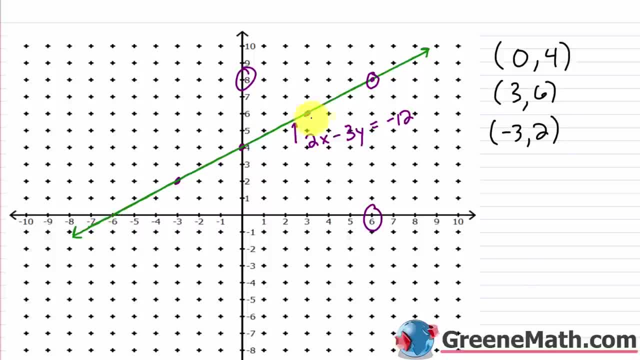 linear equation in two variables. Each and every point on that line again is an ordered pair. that is a solution to that equation. So it's a visual representation of all your solutions. Now, one of the things that I didn't explain, but I should have went. 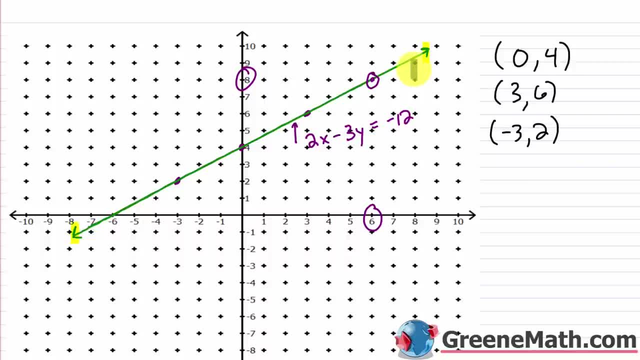 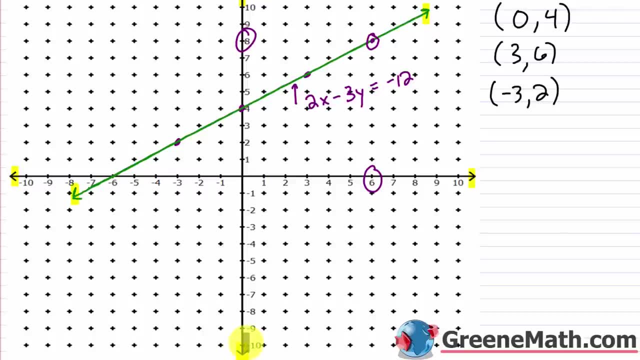 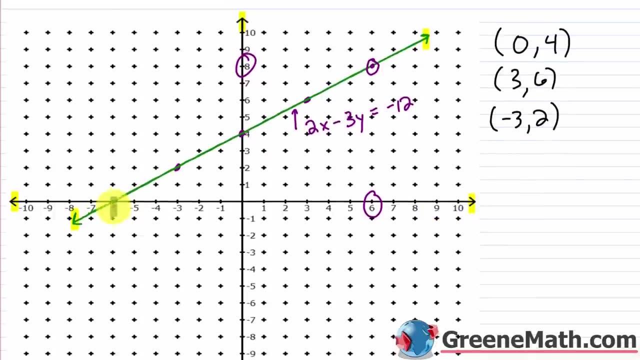 into depth on is that I drew arrows at each end. These arrows are the same as the arrows I'm drawing right here, here, here and then down here. What is that telling us? when we have an arrow, It tells us that it continues forever and ever and ever in that direction. So this: 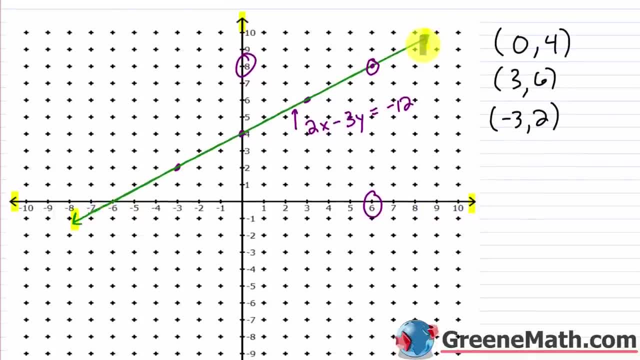 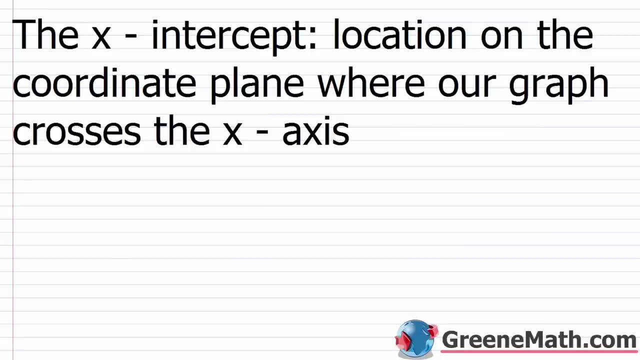 line will be the same as the arrows I'm drawing right here, here, here, and then down here, And we'll continue forever, forever and ever and ever going in this direction, and forever and ever and ever going in this direction. So that's why we put arrows at each end. All right, now let's 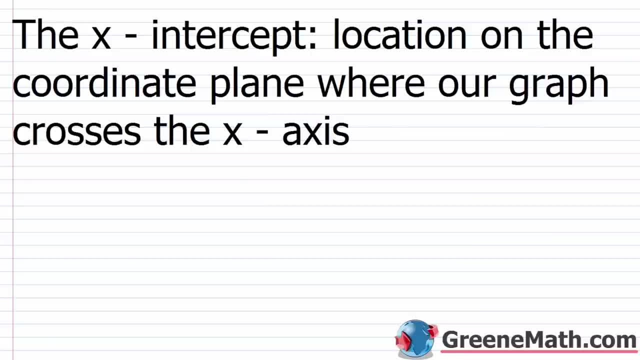 talk about a few things real quick that are very, very important. I encourage you to take notes for this section. So the x-intercept: you're going to hear about this a lot. The x-intercept is the location on the coordinate plane where our graph crosses the x-axis. Let's go back up here. 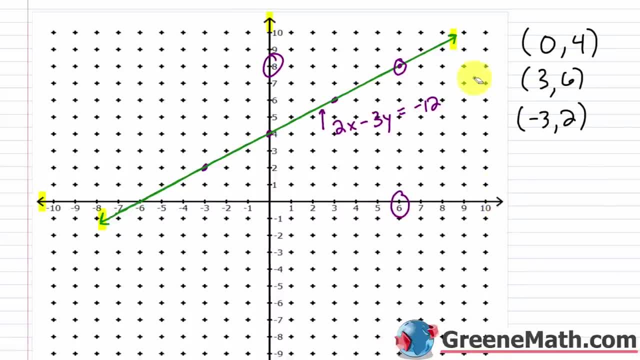 And let's look at the x-axis. So I have a lot of stuff highlighted. right now Let me unhighlight some stuff And I'm just going to highlight the x-axis. So here's the x-axis And I want you to look at. 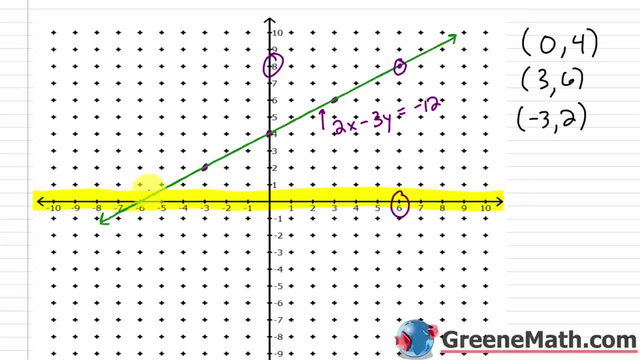 the graph And I want you to see that the line crosses through right here. This is where it crosses the x-axis. So this is known as the x-intercept. It's a point where it intercepts the x-axis And if you look at the graph, it looks like it's going to be at negative 6,0.. So negative 6,0.. This. 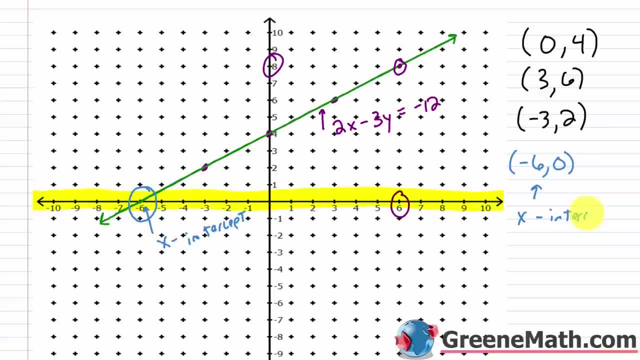 is the x-intercept And you can tell that does work out. I'd have 2 times negative 6. That's negative 12. And this negative 3y would go away because I plug in a 0 for y, Negative 3 times 0. 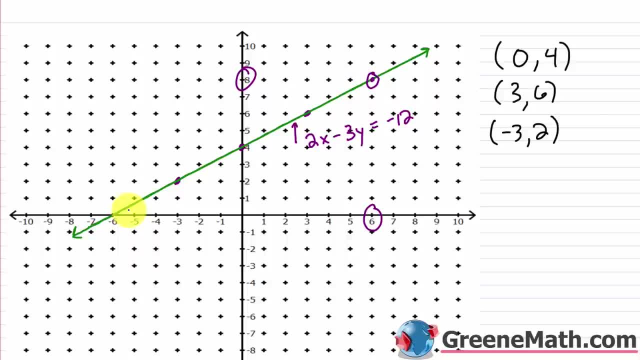 Each and every point on that line is an ordered pair that is a solution to that equation. So it's a visual representation of all your solutions. Now, one of the things that I didn't explain, but I should have went into depth on, is that I drew arrows at each end. These arrows are the same as the arrows I'm drawing right here, here, here, and then down here. 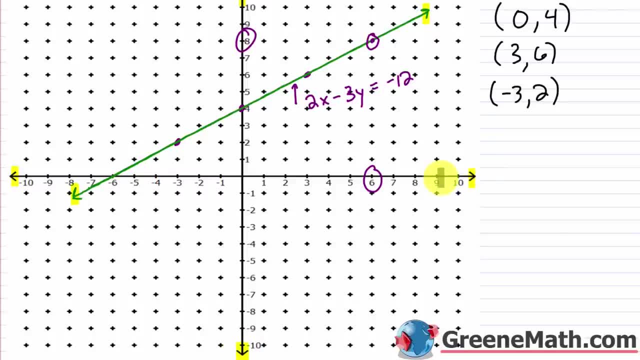 What is that telling us when we have an arrow? It tells us that it continues forever and ever and ever in that direction. So this line will continue forever. Forever and ever and ever 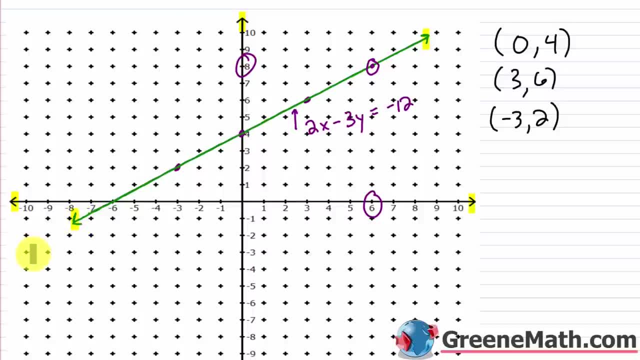 going in this direction, and forever and ever and ever going in this direction. 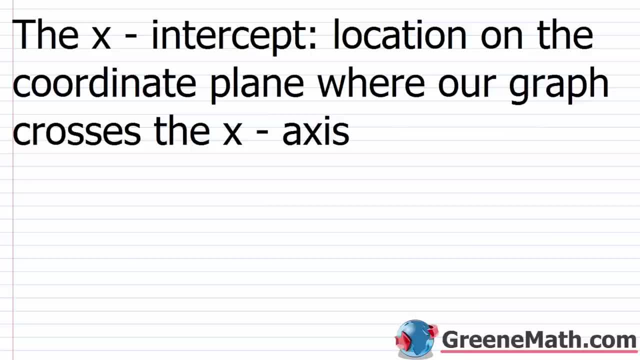 So that's why we put arrows at each end. Alright, now let's talk about 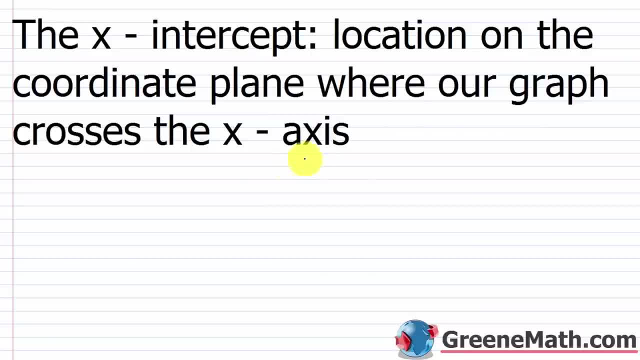 a few things real quick that are very, very important. I encourage you to take notes for this section. 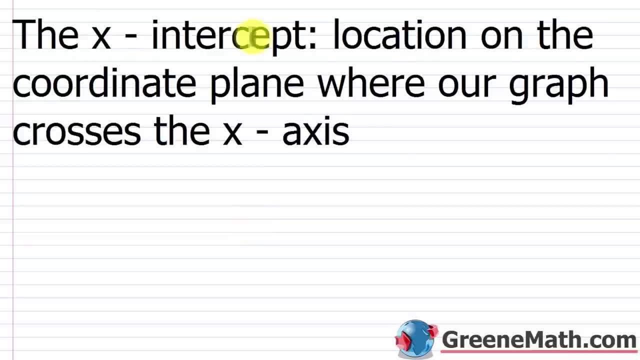 So the x-intercept. You're going to hear about this a lot. The x-intercept is the location on the coordinate plane where our graph crosses the x-axis. 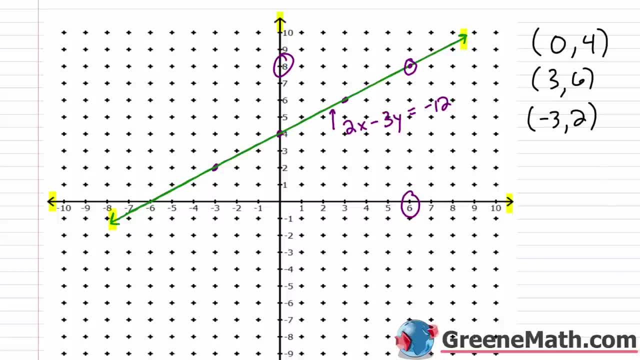 Let's go back up here. And let's look at the x-axis. So I have a lot of stuff highlighted right now. Let me un-highlight some stuff. 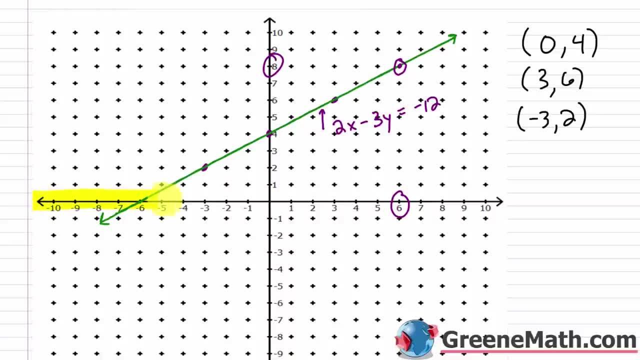 And I'm just going to highlight the x-axis. So here's the x-axis. And I want you to look at the graph, and I want you to see that the line crosses through right here. This is where it crosses the x-axis. So this is known as the x intercept. 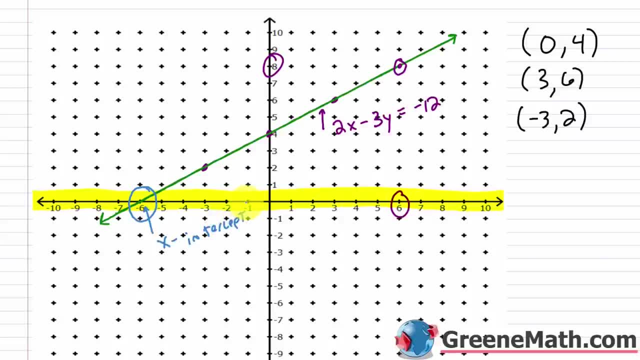 It's a point where it intercepts the x-axis. 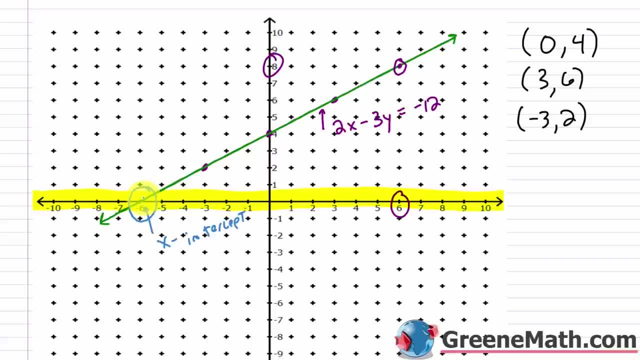 And if you look at the graph, it looks like it's going to be at . So . This is the x intercept. 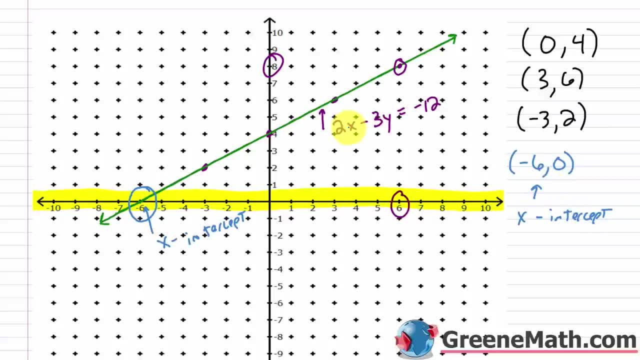 And you can tell that does work out. I'd have 2 times that's . 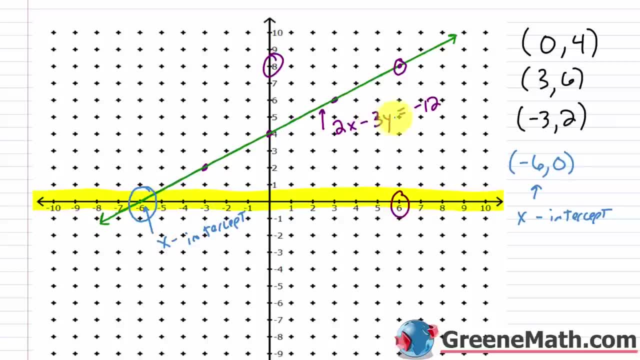 And this would go away because I plug in a 0 for y. is just 0, so that's gone. 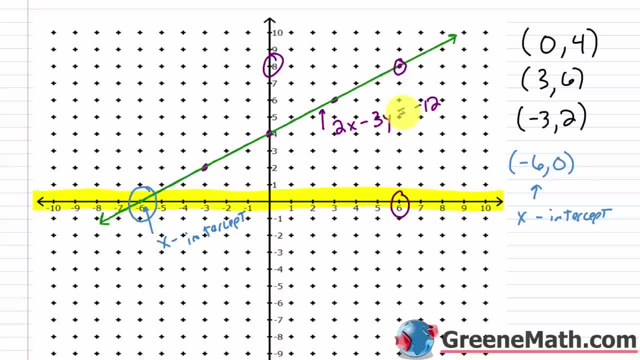 So you get equals . Now, I might want to bring your attention 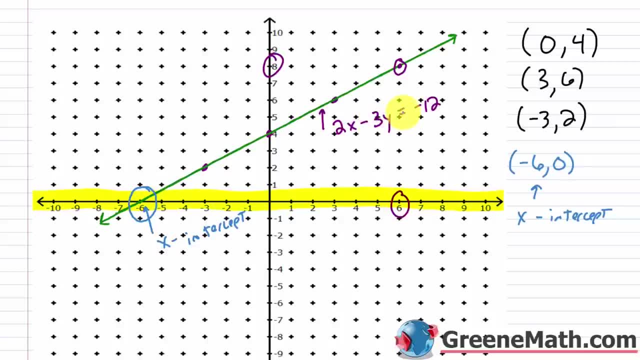 is just 0.. So that's gone. So you get negative 12 equals negative 12.. Now I might want to bring your attention to the fact that the y-location is 0. Why do you think that is? Well, if I'm on the x-axis, if I'm crossing through there, that means that 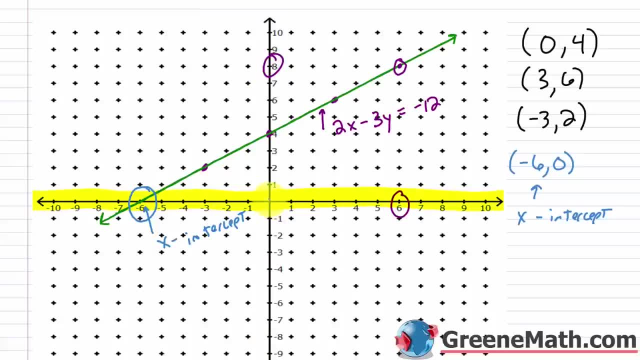 vertically, I have to be at 0 on the y-axis, Because that's where the x-axis lies Right. This is 0 on the y-axis, So to cross the x-axis, I have to be at 0 on the y-axis. Now, similarly, we have this: 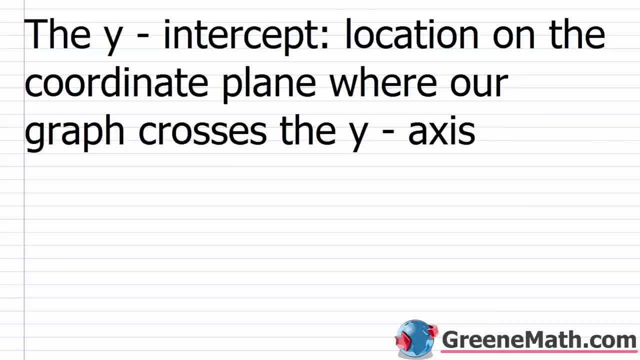 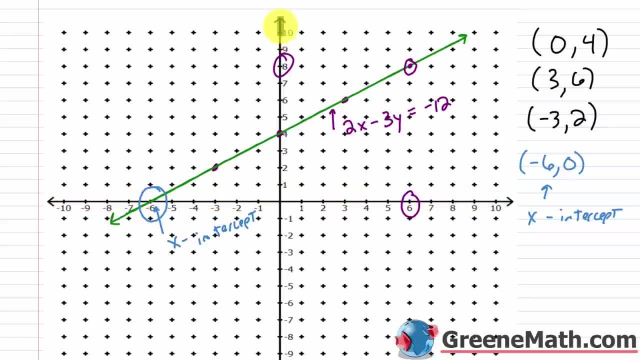 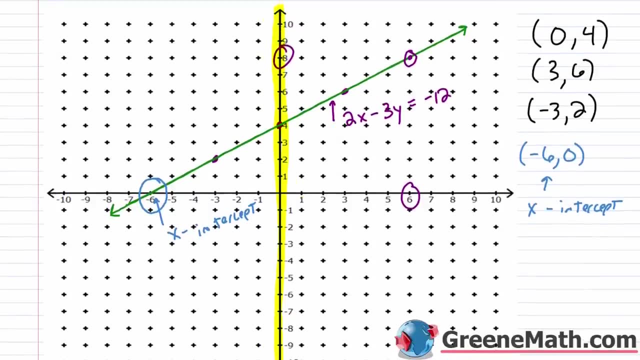 thing called the y-intercept. This is the location on the coordinate plane where our graph crosses the y-axis. So let me unhighlight all this stuff. So the y-axis is here. This is the y-axis. So where does the graph cross there? Well, it crosses right here, At 0 for the x-location and 4 for the y-location. So this is your y-intercept. 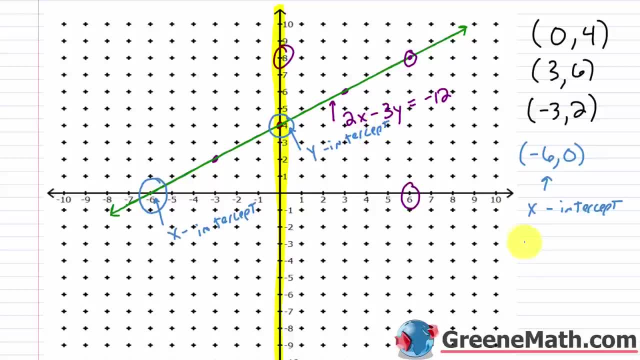 And this occurs at 0, 4.. This is the y-intercept, And does that work out? Well, yeah, If I plug in a 0 for x, this would go away. I'd have negative 3 times 4. That is negative 12.. So I get negative. 12 equals negative 12.. 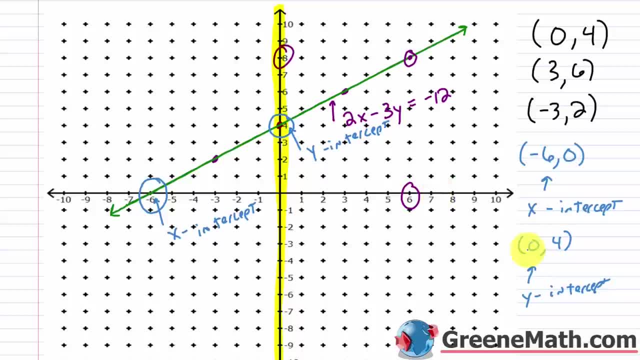 Now, one thing again I want to call your attention to is notice how your x-coordinate is 0. Because if I look at this horizontal axis, the x-axis, it has to be 0 for me to impact the y-axis. 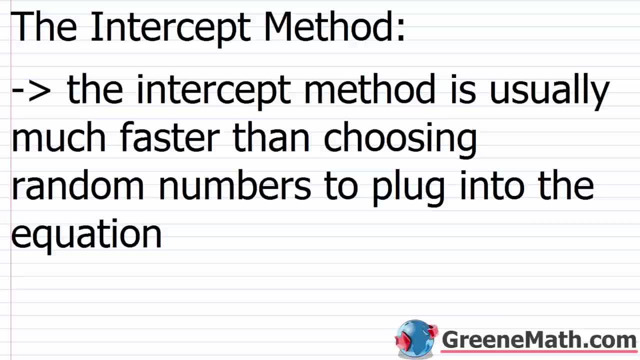 So this leads us to another method, And this is called the intercept method. You'll probably hear about this in your class class. So the intercept method is usually much faster than choosing random numbers to plug into the equation. So we begin by finding the x and y intercepts, and then we also like 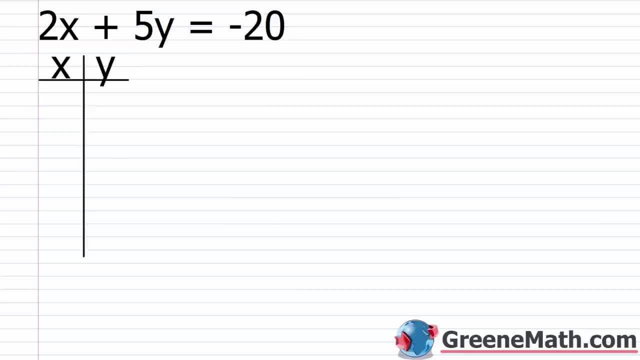 one additional point for a check. So how do we find the x-intercept? Well, again, I told you, if you want to cross the x-axis, y has to be 0. If I look at the coordinate plane, y has to be 0 to cross the x-axis. So for the x-intercept, y is 0.. For the y-intercept: 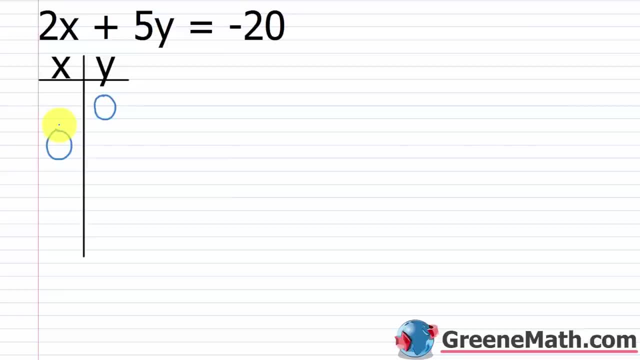 x is 0. So that's how you find your two intercepts. Again, if I want the x-intercept, the opposite one- y- is 0.. If I want the y-intercept, the opposite one- x is 0.. So this would be the. 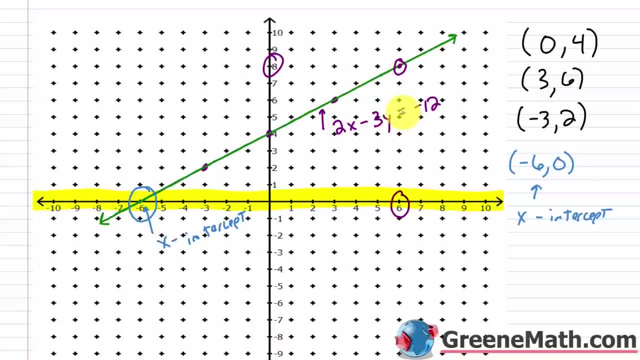 to the fact that the y location is 0. Why do you think that is? Well, if I'm on the x-axis, if I'm crossing through there, that means that vertically I have to be at 0 on the y-axis. Because that's where the x-axis lies. This is 0 on the y-axis. 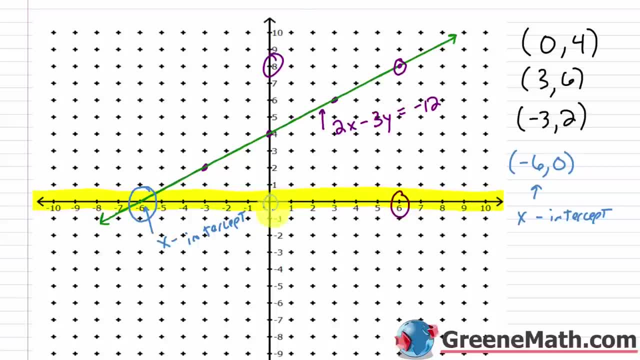 So to cross the x-axis, I have to be at 0 on the y-axis. 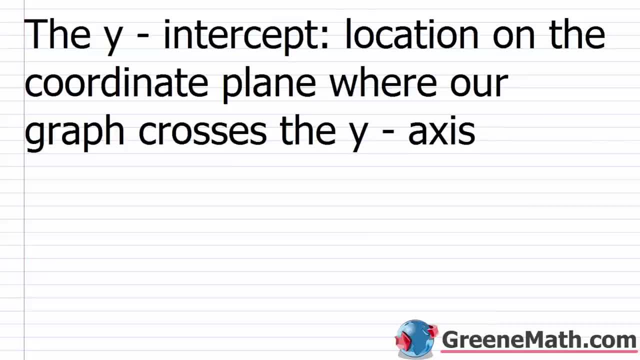 Now similarly, we have this thing called the y intercept. 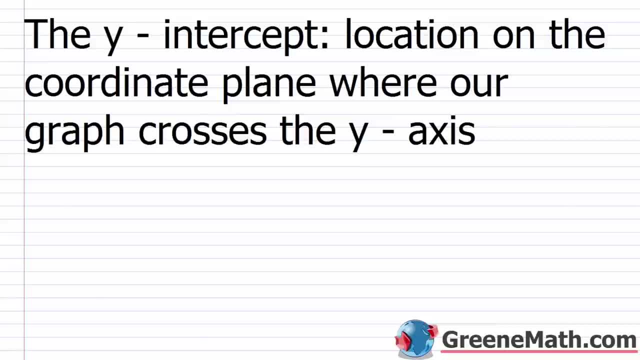 This is the location on the coordinate plane where our graph crosses the y-axis. 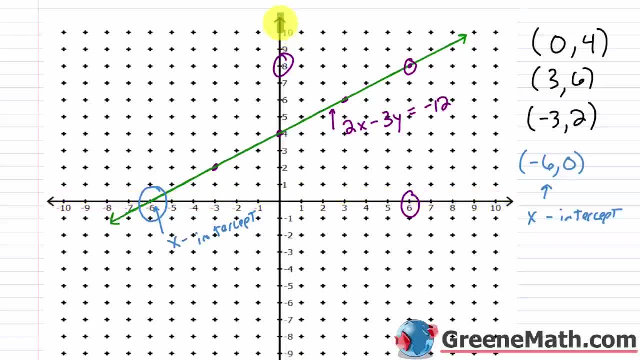 So let me unhighlight all this stuff. So the y-axis is here. This is the y-axis. 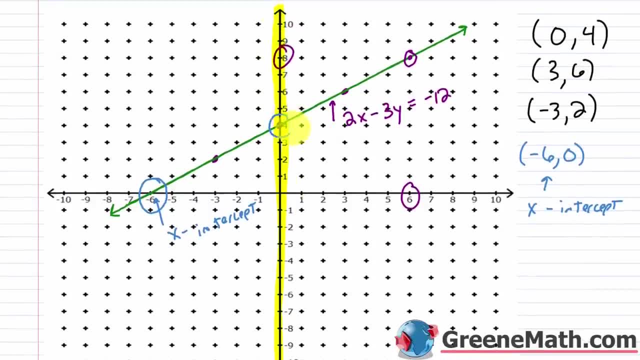 So where does the graph cross there? It crosses right here. At 0 for the x location and 4 for the y location. So this is your y intercept. And this occurs at . 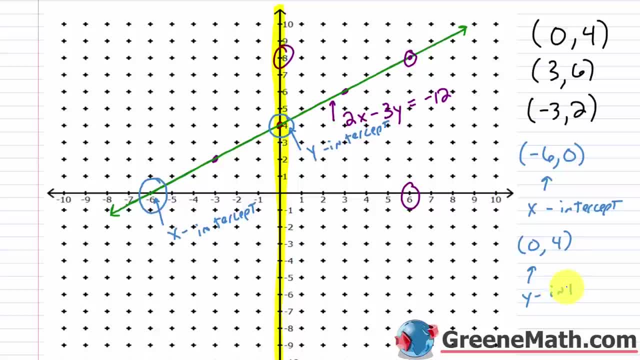 This is the y intercept. 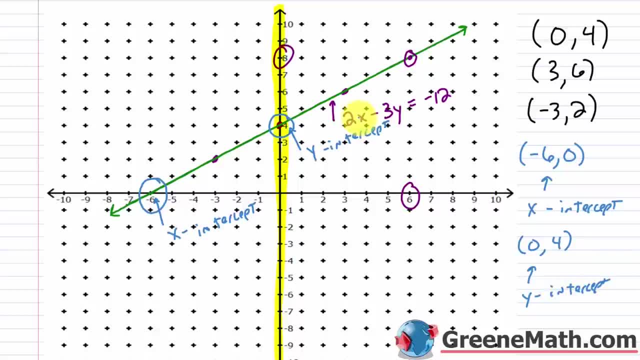 And does that work out? Well yeah, if I plug in a 0 for x, this would go away. I'd have negative 3 times 4. That is negative 12. So I'd get negative 12 equals negative 12. 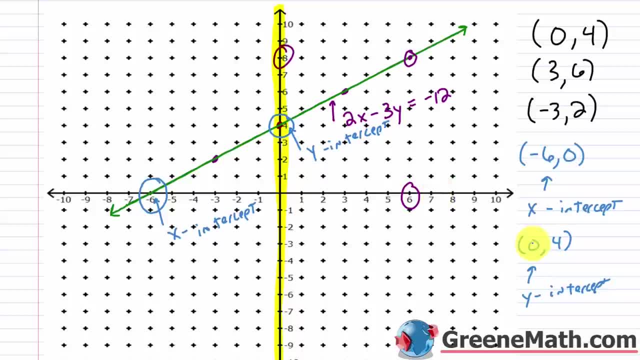 Now one thing again I want to call your attention to is notice how your x coordinate is 0. 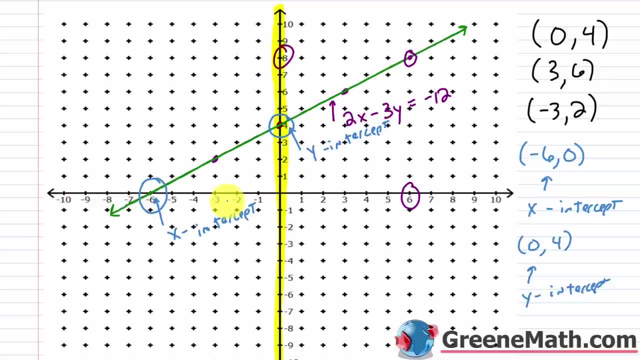 Because if I look at this horizontal axis, the x-axis, it has to be 0 for me to impact the y-axis. 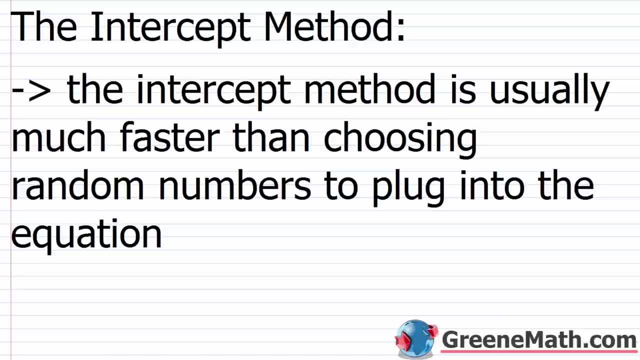 So this leads us to another method. And this is called the intercept method. You'll probably hear about this in your class. 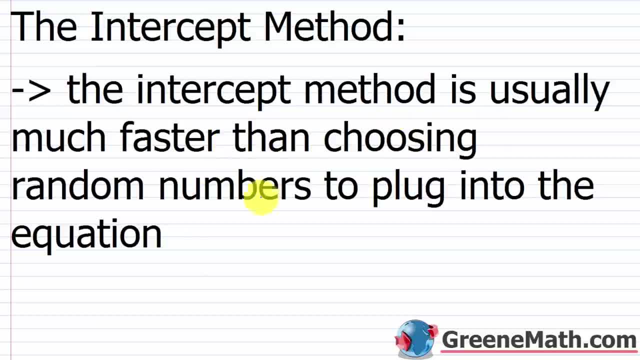 So the intercept method is usually much faster than choosing random numbers to plug into the equation. 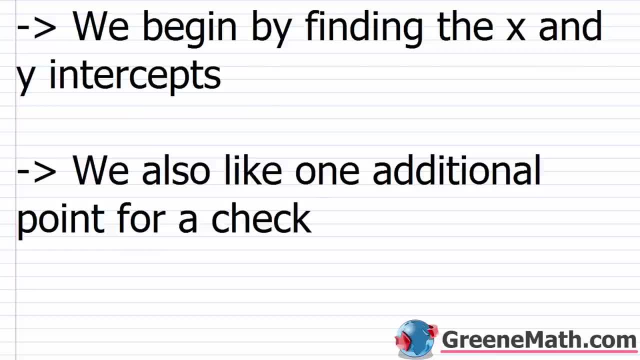 So we begin by finding the x and y intercepts. And then we also like one additional point for a check. 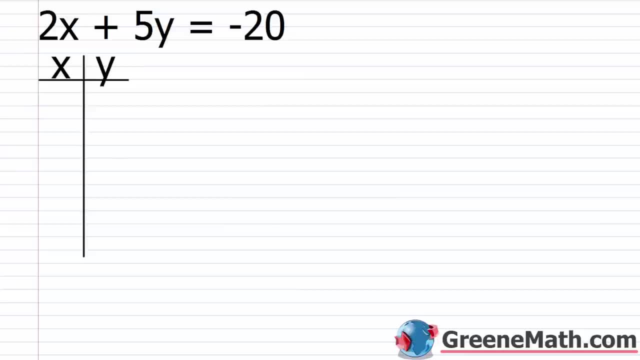 So how do we find the x-intercept? Well again, I told you if you want to cross the x-axis, y has to be 0. If I look at the coordinate plane, y has to be 0 to cross the x-axis. 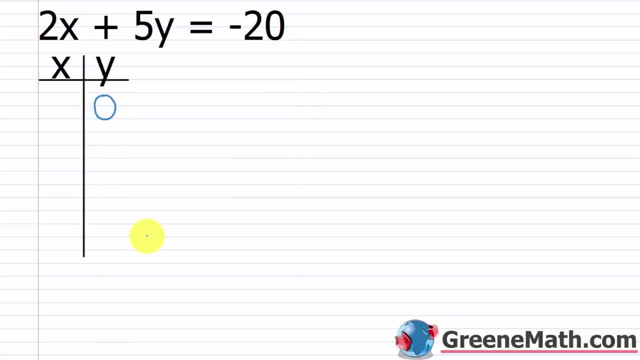 So for the x-intercept, y is 0. For the y-intercept, x is 0. So that's how you find your two intercepts. 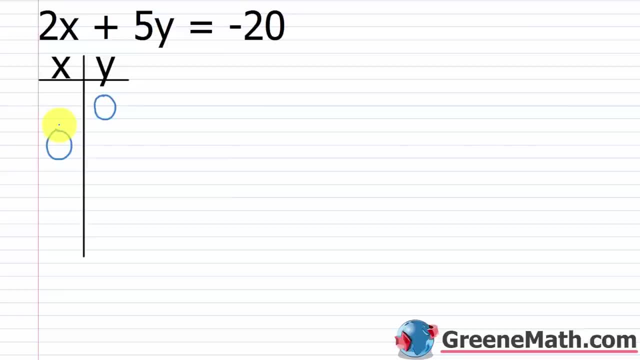 Again, if I want the x-intercept, the opposite one, y, is 0. If I want the y-intercept, the opposite one, x, is 0. So this would be the x-intercept. 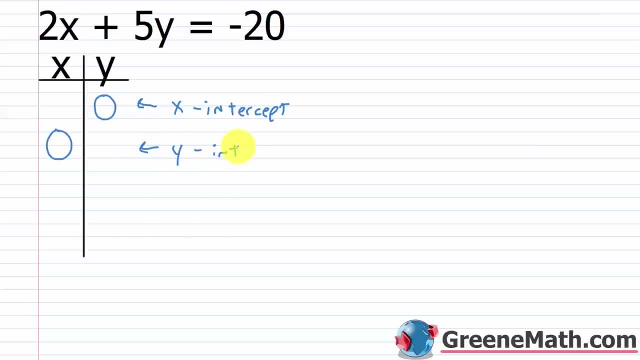 And this would be the y-intercept. 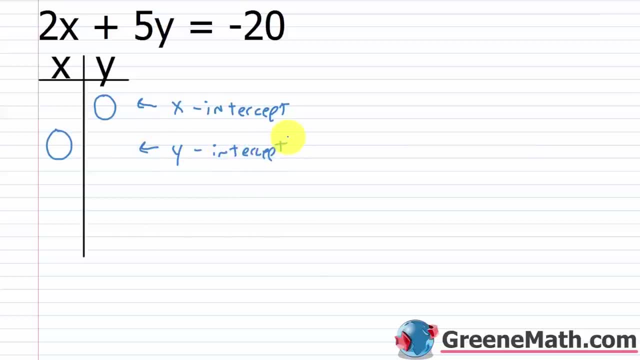 And then we'll get a third point as a check. 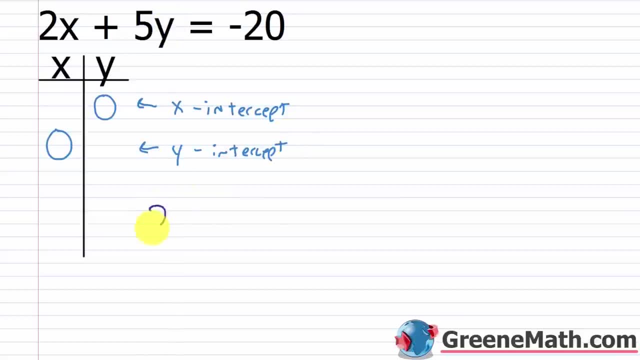 So let's go ahead and plug in a 0 for y. We'd have 2x plus, 5 times 0 is just 0, so I can just have 2x. This equals negative 20. 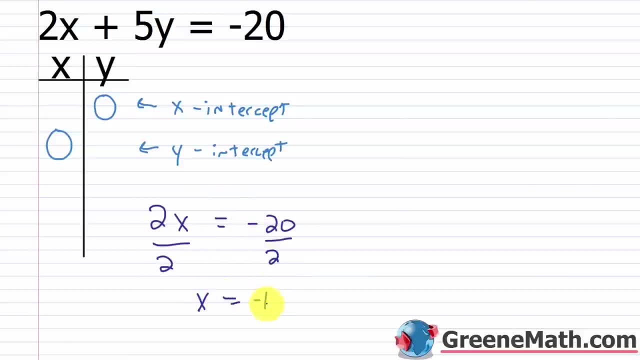 Divide both sides by 2. And you get x equals negative 10. 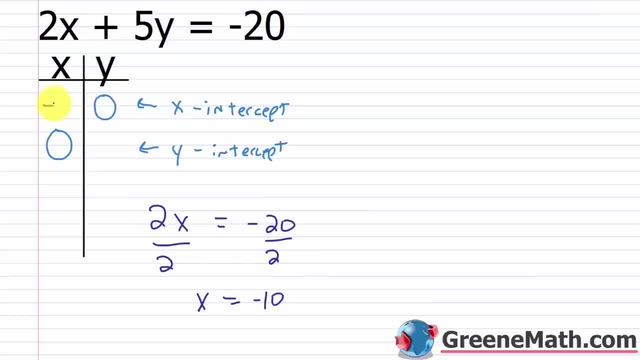 So if y is 0, x is negative 10. 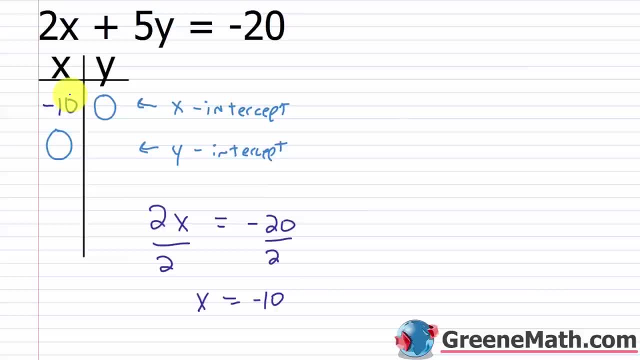 And look how easy that was. When you work with 0, you plug it in, it makes things disappear. It makes your work a lot simpler. That's why this intercept method is usually a little faster. 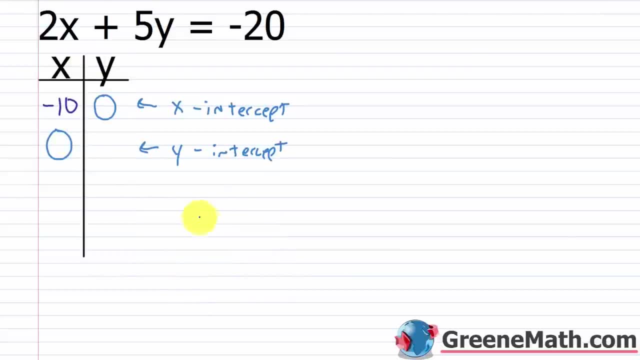 Now the other one, we're going to plug a 0 in for x. So this is the y-intercept. So 2 times 0, plus 5y equals negative 20. And again, I can just get rid of this. So 5y equals negative 20. Divide both sides by 5. You get y equals negative 4. So now I've got two ordered pairs. But again, I like 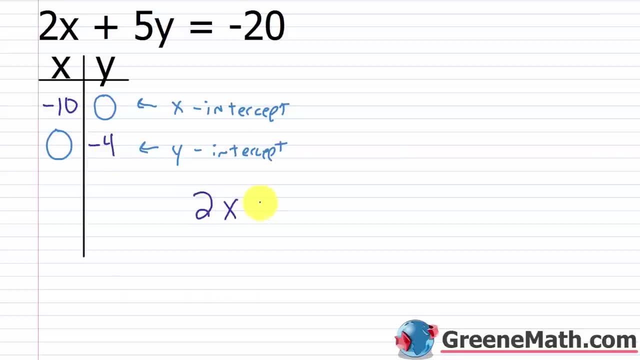 So what am I going to plug in for x? Well, if I look at this equation, 2x plus 5y equals negative 20. Again, if I think about this, whatever I plug in for x, I'm going to end up moving this over here. Right now, negative 20 is divisible by 5. So if I've got to pick something that I plug in here and move it over here to where it's still going to be divisible by 5, otherwise I'm not going to end up with an integer. So one thing you can think about is, if I multiply 2 times 5, 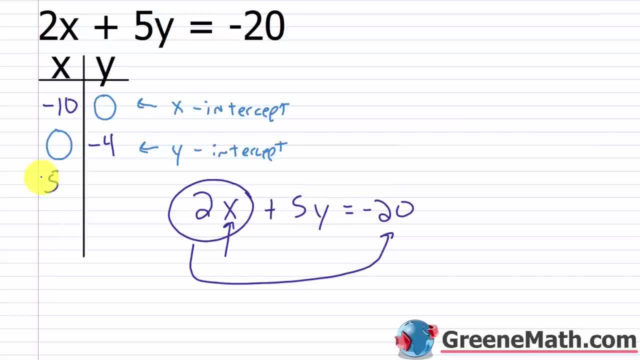 2 times 5, that would give me 10. Now, if I subtract 10 away from negative 20, I'm going to get negative 30, and that's divisible by 5. So that would work out. 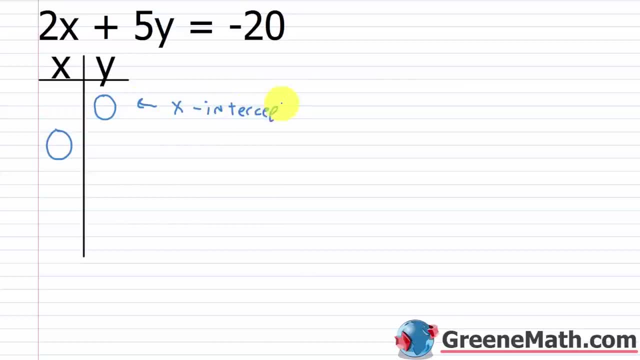 x-intercept and this would be the y-intercept. And then we'll get a third point as a check. Let's see. So let's go ahead and plug in a 0 for y. You'd have 2x plus 5 times 0 is just 0, so 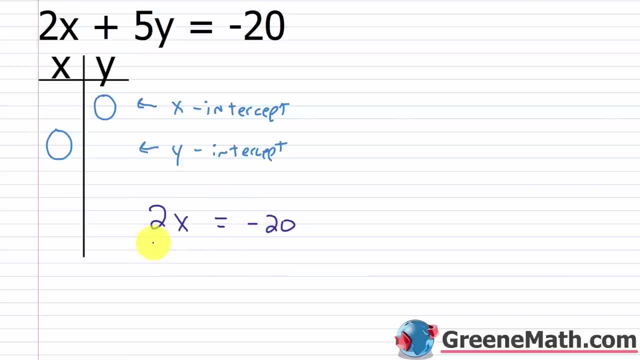 I can just have 2x. This equals negative 20.. Divide both sides by 2, and you get x equals negative 10.. So if y is 0,, x is negative 10.. And look how easy that was When you work. 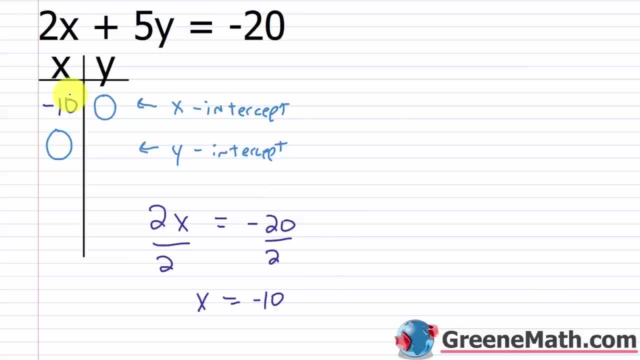 with 0, you plug it in, it makes things disappear, makes your work a lot simpler. That's why this intercept method is usually a little faster. All right, now the other one. we're going to plug a 0 in for x. So this is the y-intercept. So 2 times 0 plus 5y equals negative. 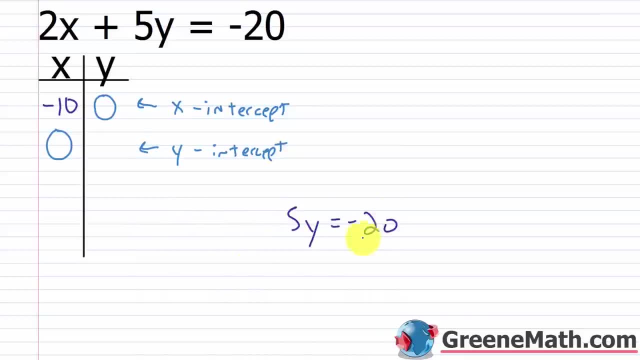 20. And again I can just get rid of this. So 5y equals negative 20. Divide both sides by 5. You get y equals negative 4. So now I've got two ordered pairs, But again I like a third one for a check. So what am? 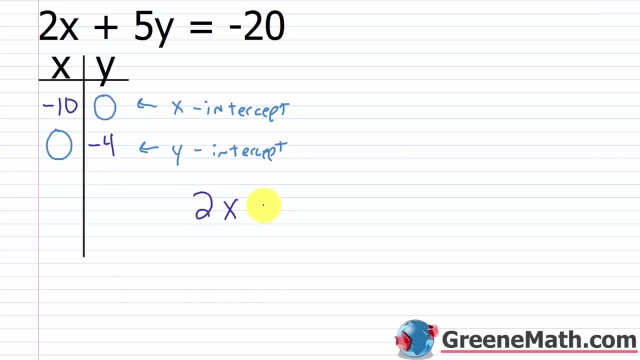 I going to plug in for x. Well, if I look at this equation, 2x plus 5y equals negative 20. 0. So if I think about this, whatever I plug in for x, I'm going to end up moving this. 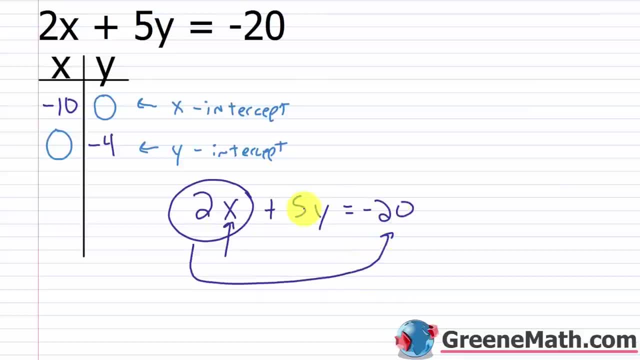 over here. Right now, negative 20 is divisible by 5.. So if I've got to pick something that I plug in here and move it over here to where it's still going to be divisible by 5, otherwise I'm not going to end up with an integer. 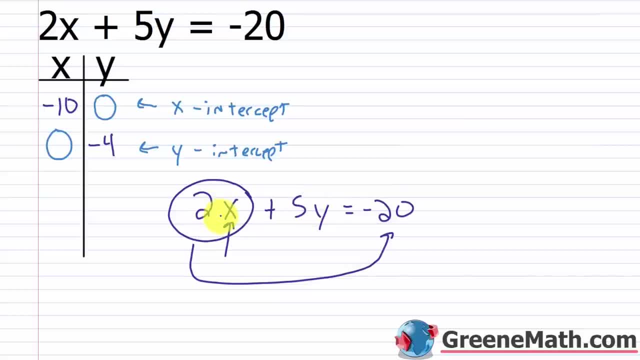 So one thing you can think about is if I multiply 2 times 5, 2 times 5,, that would give me 10.. Now if I subtract 10 away from negative 20,, I'm going to get negative 30, and that's the. 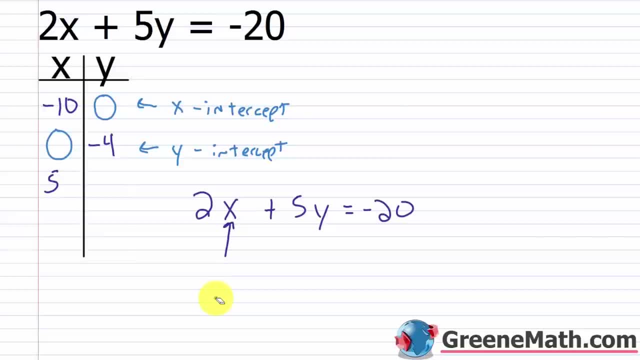 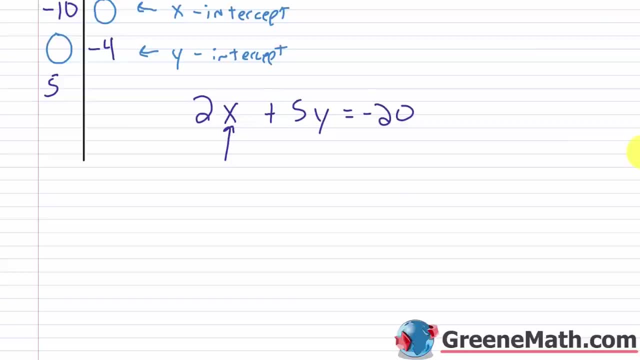 same thing. So again, you want to kind of think about that before you start plugging in random numbers, because if you end up with a non-integer, you just wasted your time, right, It's very hard to plot that. So you plug in a 5 here You would have 2 times 5, or 10, plus 5y equals negative 20.. 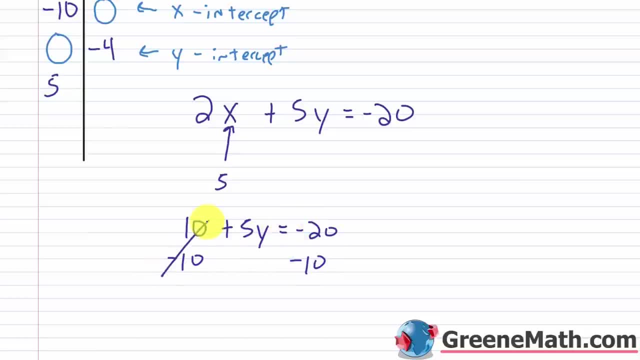 I would subtract 10 away from each side of the equation. That's gone. I'll have 5y is equal to negative 30. Divide both sides by 5.. I'm going to get that y is equal to negative 6.. 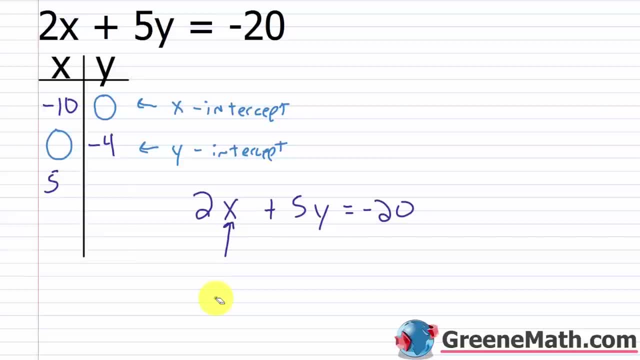 So again, you want to kind of think about that before you start plugging in random numbers, because if you end up with a non-integer, you just wasted your time, right? It's very hard to plot that. 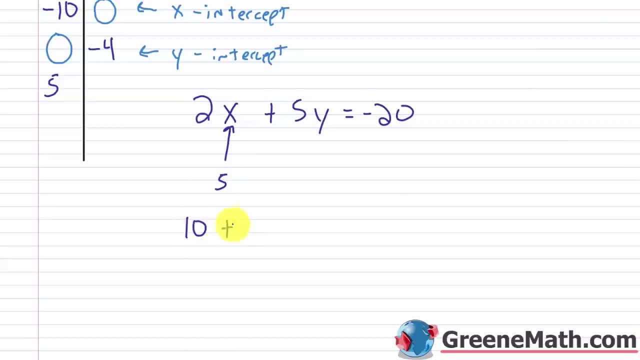 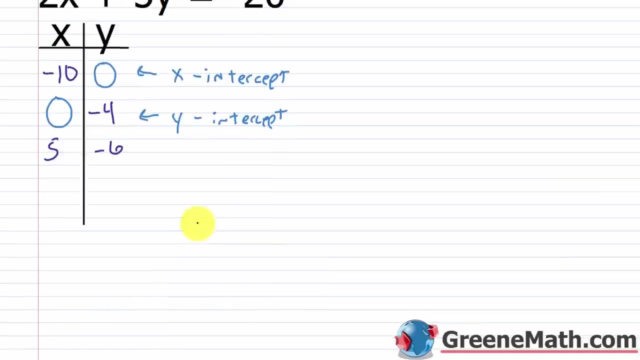 So you plug in a 5 here. You would have 2 times 5, or 10, plus 5y equals negative 20. I would subtract 10 away from each side of the equation. That's gone. I'll have 5y is equal to negative 30. Divide both sides by 5. I'm going to get that y is equal to negative 6. Alright, so I have three ordered pairs. I have negative 10, comma 0. I have 0, comma negative 4. 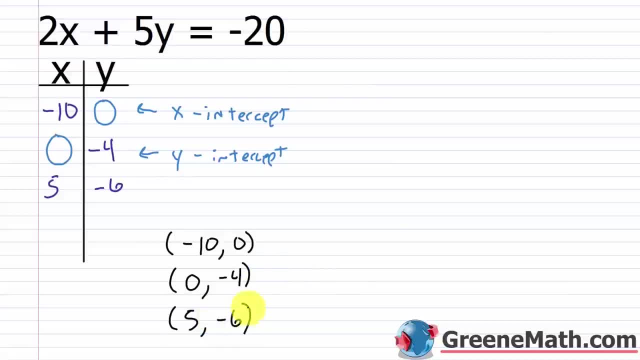 And I have 5, comma negative 6. So let's plot these points 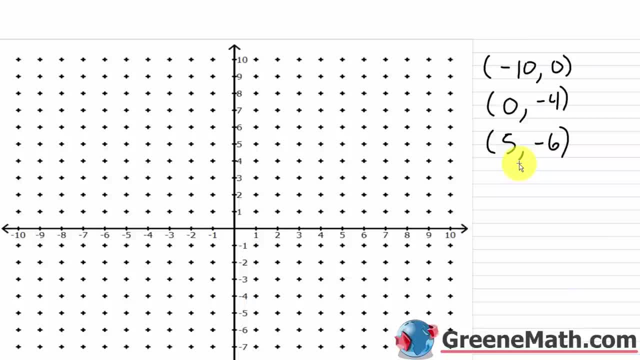 on the coordinate plane, and then we'll draw a straight line through them. Alright, so let's begin 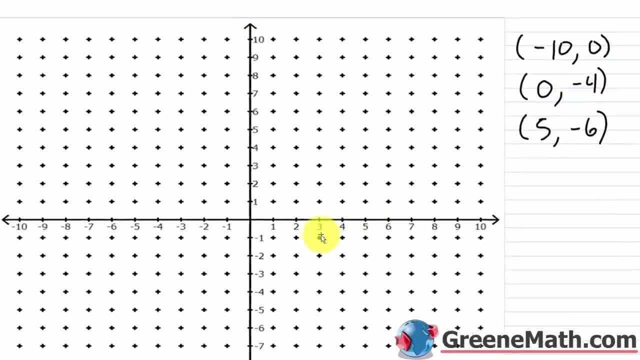 with negative 10, comma 0. So that's all the way to the left 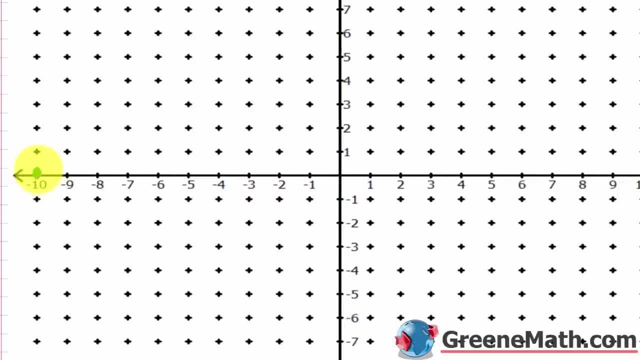 on the x-axis. So way over here. This is negative 10, 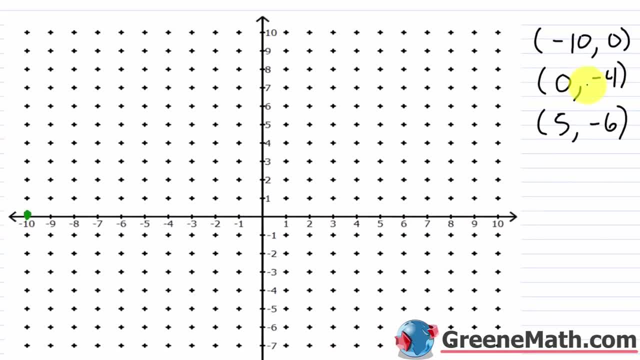 comma 0. Then I have 0, comma negative 4. So that's down 4 on the y-axis. 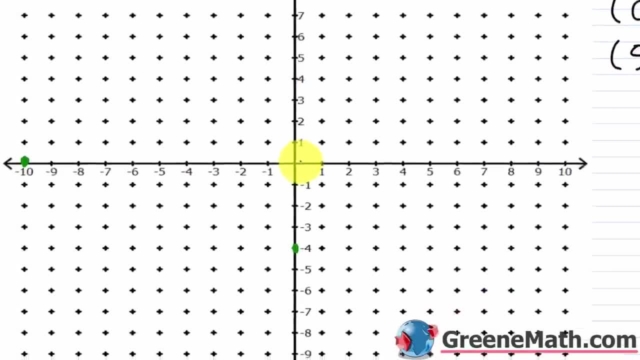 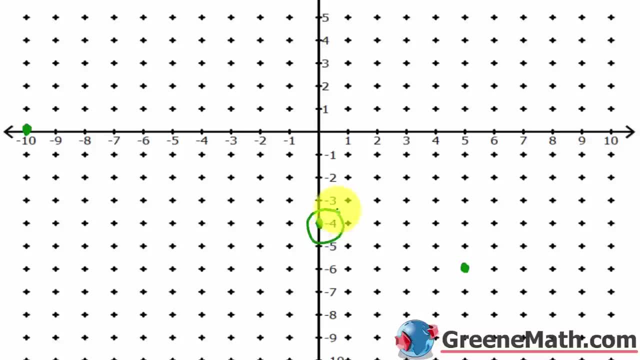 And then I have 5, comma negative 6. So I go to the right 5 and down 6. And you can see that when I draw a straight line through it, the line's going to cross through here, which the x-location is 0. So it's crossing through the y-axis. This is the y-intercept. 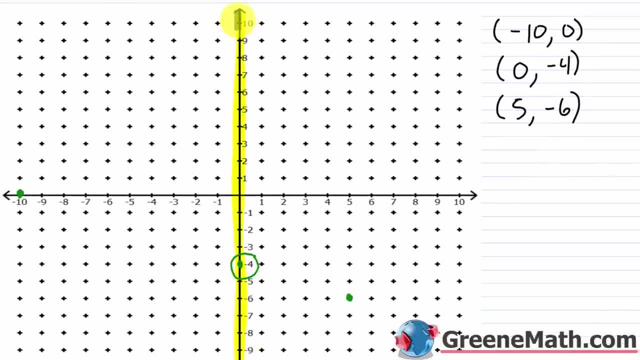 Alright, x-location is 0 at that point. 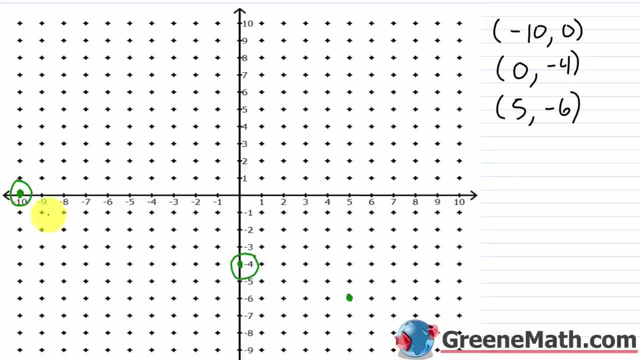 And then notice how it's also going to impact the x-axis here 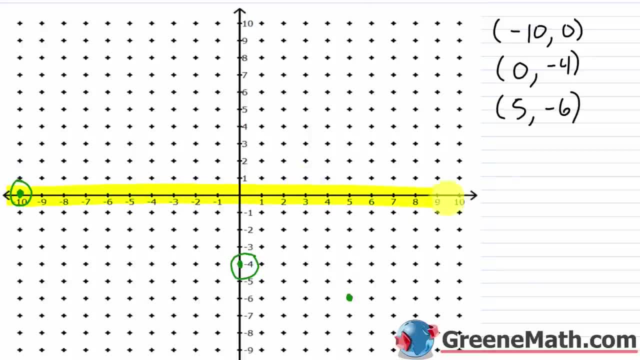 where y is going to be 0. Okay, y is going to be 0. That's your x-intercept. 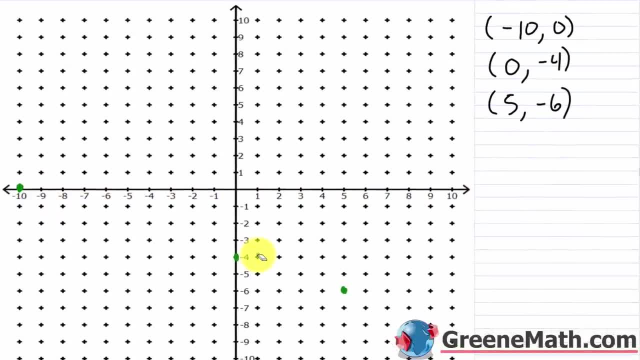 Alright, so let's draw a straight line through these points now. 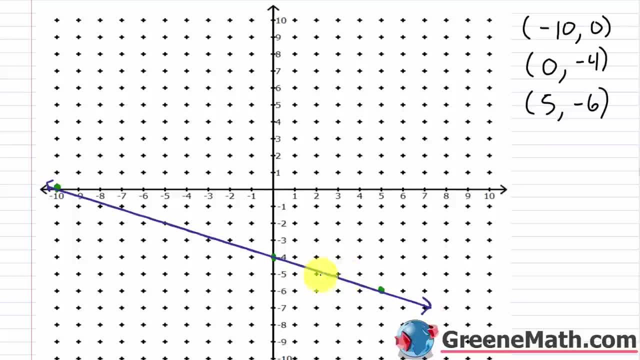 Okay, so put arrows at each end. And the line's not perfect, but it'll do for what we're trying to accomplish here. 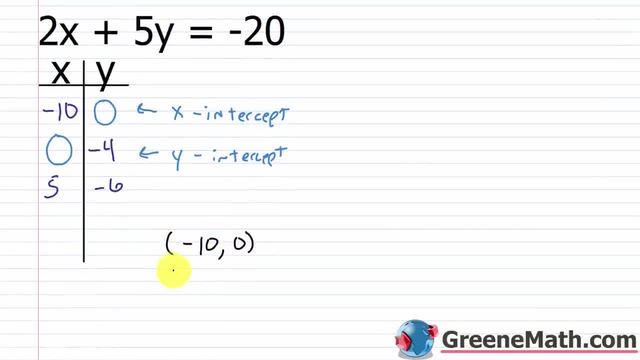 So I have 3 ordered pairs. I have negative 10, comma 0.. I have 0, comma negative 4.. And I have 5, comma negative 6.. So let's plot these points on the coordinate plane and then we'll draw a straight line. 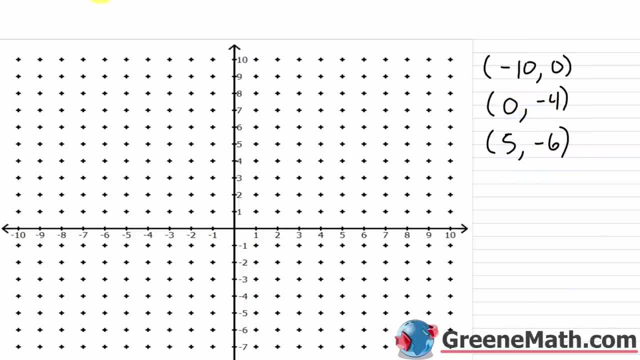 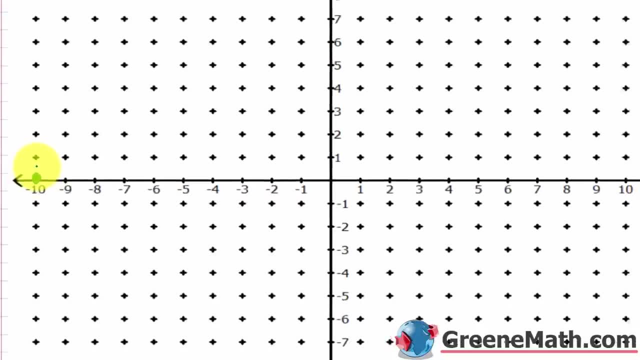 through them. All right, so let's begin with negative 10, comma 0.. So that's all the way to the left on the x-axis. so way over here. This is negative 10, comma 0.. Then I have 0, comma negative. 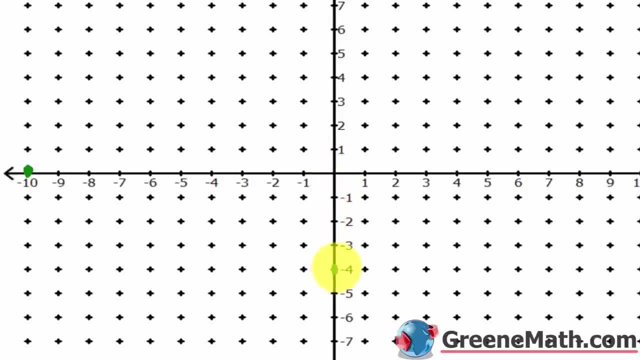 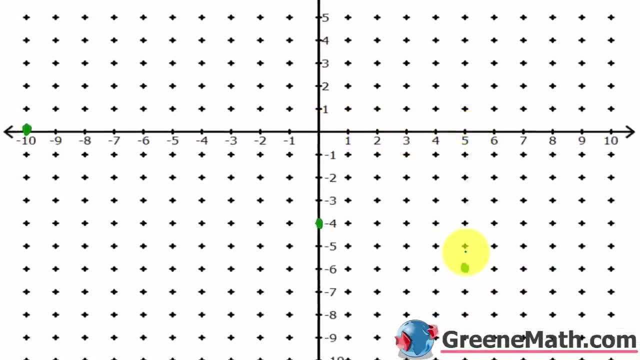 4.. So that's down 4 on the y-axis, And then I have 5.. 5, comma, negative 6.. So I go to the right 5 and down 6.. And you can see that when I draw a straight line through it, the line's going to cross. 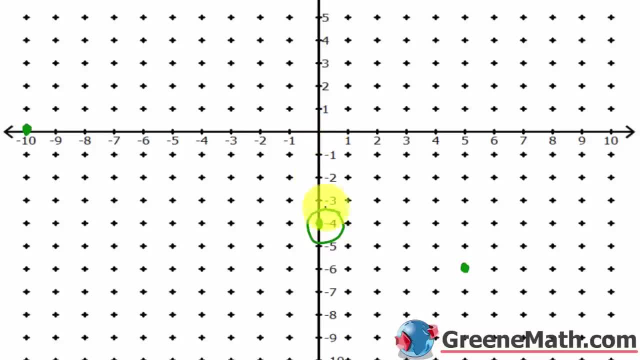 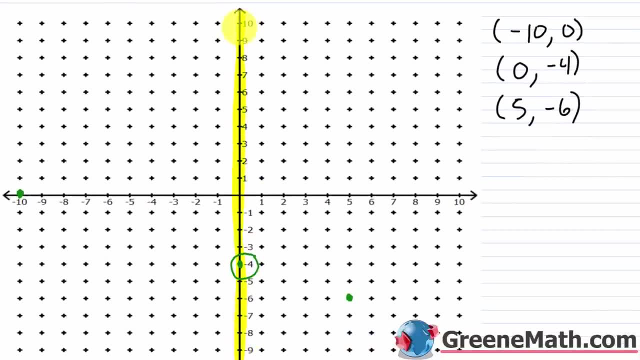 through here, which the x-location is 0.. So it's crossing through the y-axis. This is the y-intercept. All right, x-location is 0 at that point. And then notice how it's also going to impact the x-axis here, where y is going to be 0.. 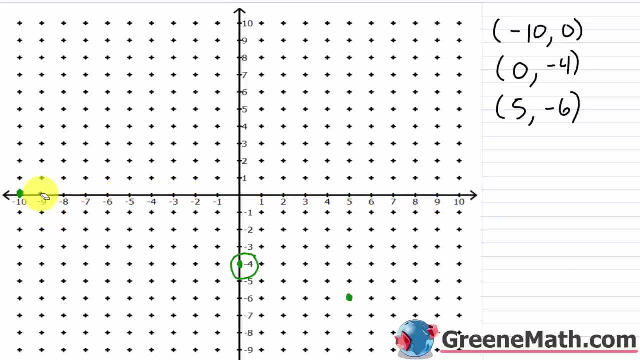 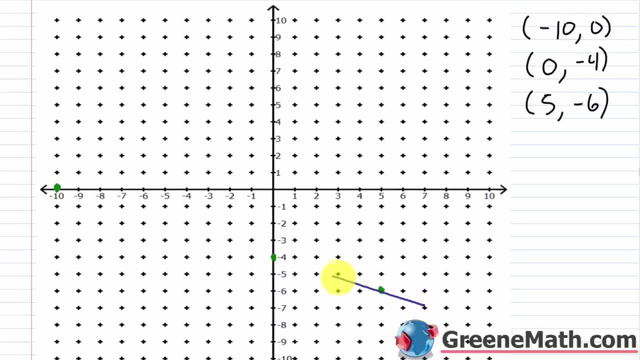 Okay, y is going to be 0.. And then the y-intercept. All right, so let's draw a straight line through these points now. Okay, so put arrows at each end And the line's not perfect, but it'll do for what we're trying to accomplish here. 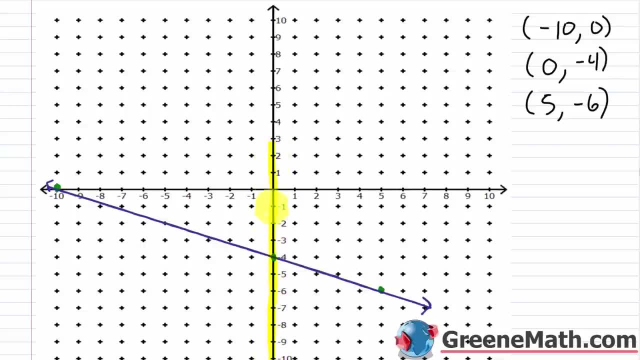 And again, look at where this line crosses the y-axis And call your attention to that Right here, at the point 0,, comma negative 4.. So the x-location is 0. And notice how on your horizontal axis, you're in the center at 0.. 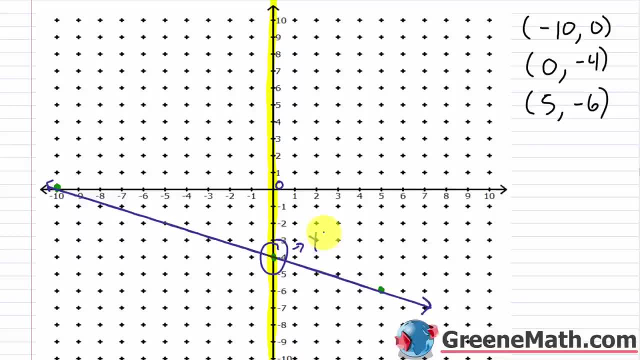 So that's your y-intercept, This is the y-intercept, And again x is 0 at that spot. Then when we look at our x-intercept, again, that's the spot where our line crosses the x-axis. That's going to be right here. 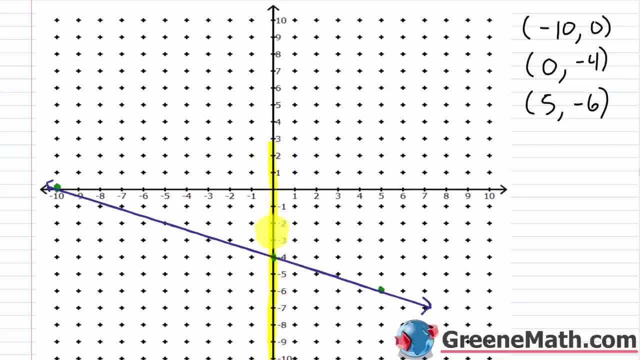 And again, look at where this line crosses the y-axis. And call your attention to that. 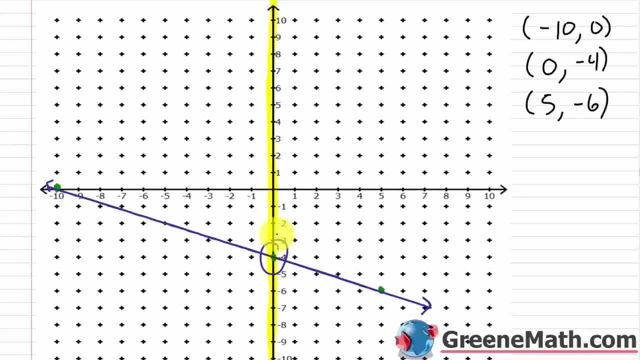 Right here, at the point 0, comma negative 4. So the x-location is 0. And notice how on your horizontal axis, your x-location is in the center, at 0. 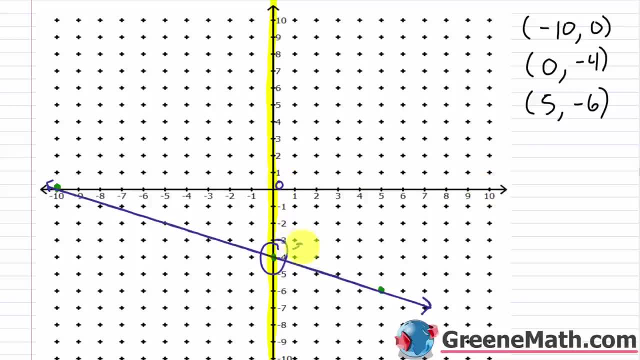 So that's your y-intercept. This is the y-intercept. 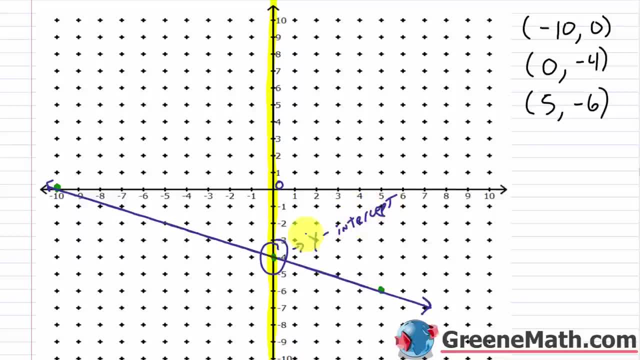 And again, x is 0 at that spot. 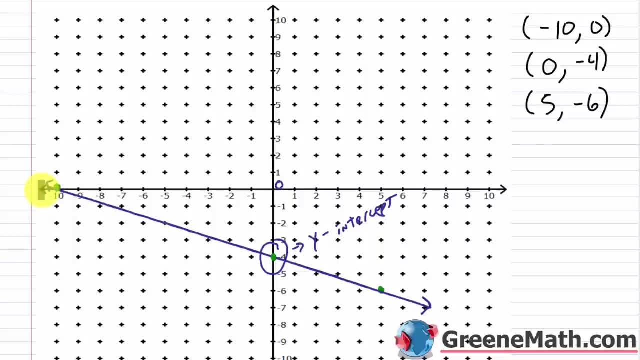 Then when we look at our x-intercept, again, that's the spot where our line crosses the x-axis. That's going to be right here. 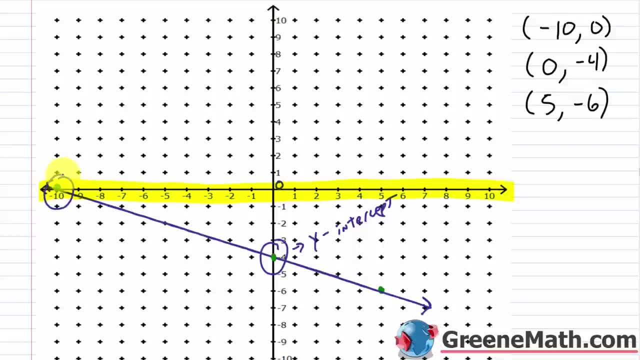 That's at negative 10, comma 0. Notice how your vertical location, your location on the y-axis, is 0 there. And let me just label this real quick as the x-intercept. And let me just label this line as the graph for 2x plus 5y equals negative 20. And again, long story short, the main thing I want you to understand here is that for your x-intercept, y needs to be 0. So just plug in a 0 for y, solve for x, 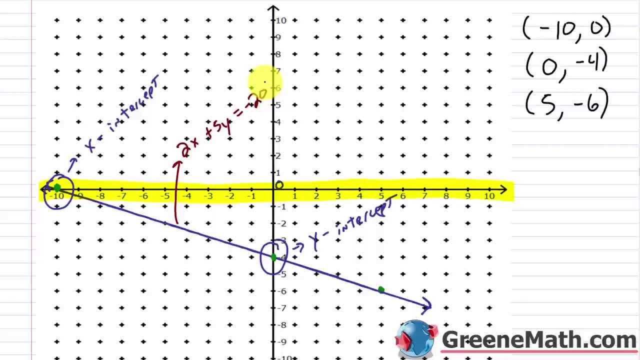 that's your x-intercept. For the y-intercept, x needs to be 0. So plug in a 0 for x, solve for y, that's how you get your y-intercept. 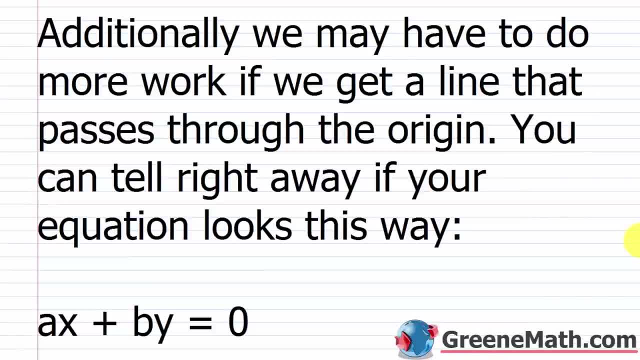 So most of the examples you're going to see, especially at first, are going to be like the previous two. But occasionally, you're going to have to do a little bit more work because you're going to get a line that passes through the origin. 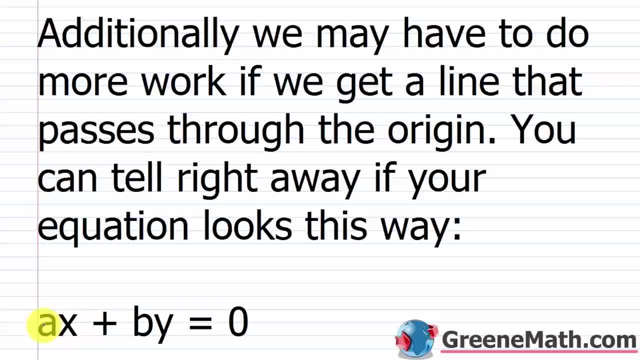 You can tell right away if your equation looks like this. 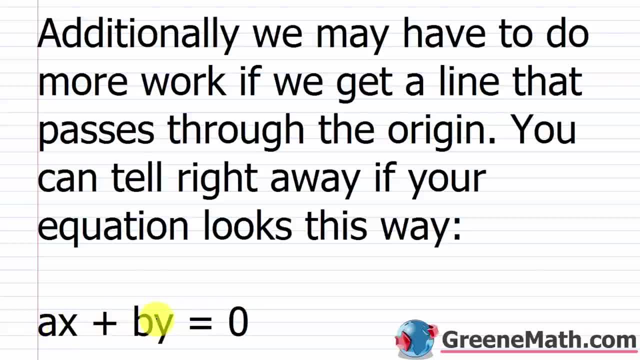 ax plus by equals 0. So some number times x plus some number times y equals 0. 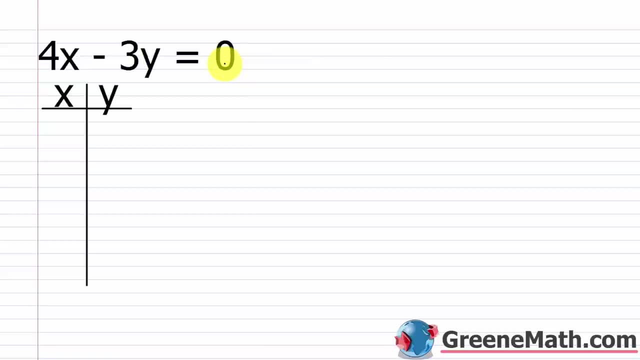 So we have an example here. 4x minus 3y equals 0. So the reason it's additional work is because if you try to use your intercept method here, the x and the y-intercept occur at the same point, which is 0 comma 0. The line passes through that 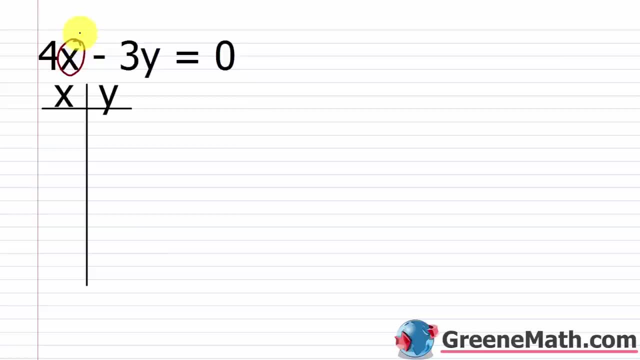 because that's the origin. If I plugged in a 0 for x, you can think about this term just going away. You'd have negative 3y equals 0. Well the only way negative 3y can equal 0 is if y is 0. So 0 comma 0 is a point on that line. 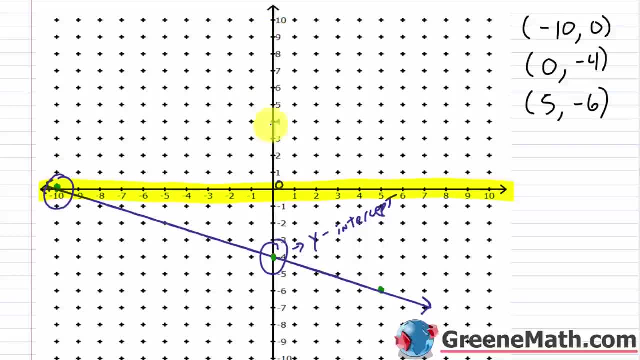 That's at negative 10, comma 0.. Okay, So now your vertical location, your location on the y-axis, is 0 there, And let me just label this real quick as the x-intercept, And let me just label this line as the graph, for 2x plus 5y equals negative 20.. 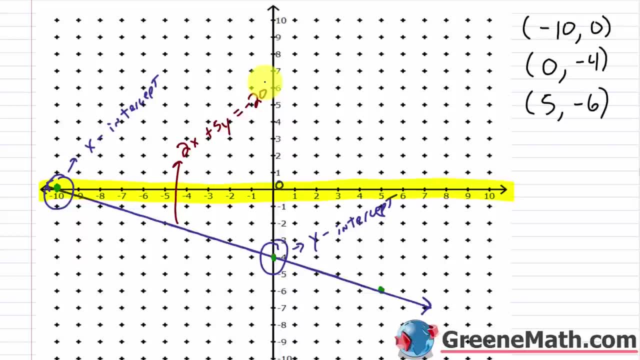 And again, long story short, the main thing I want you to understand here is that for your x-intercept, y needs to be 0. So just plug in a 0 for y, solve for x. That's your x-intercept. 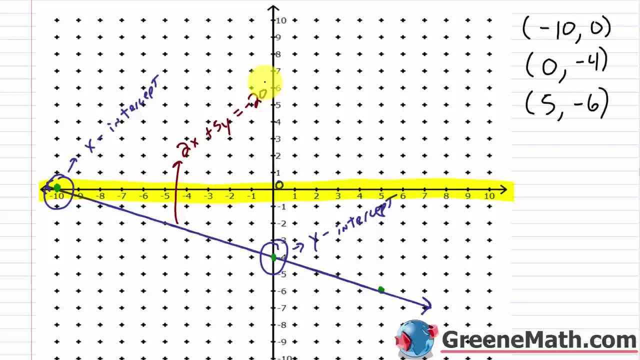 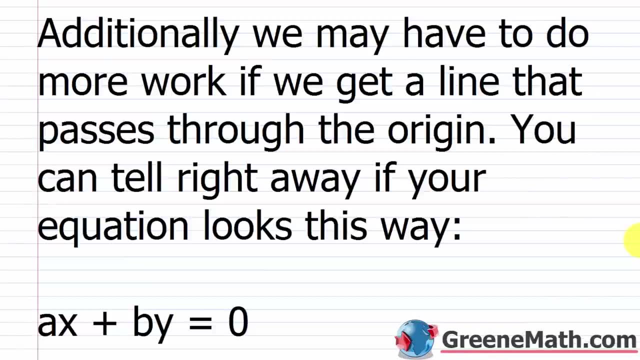 For the y-intercept, x needs to be 0. Okay, So plug in a 0 for x, solve for y. That's how you get your y-intercept. So most of the examples you're going to see, especially at first, are going to be like: 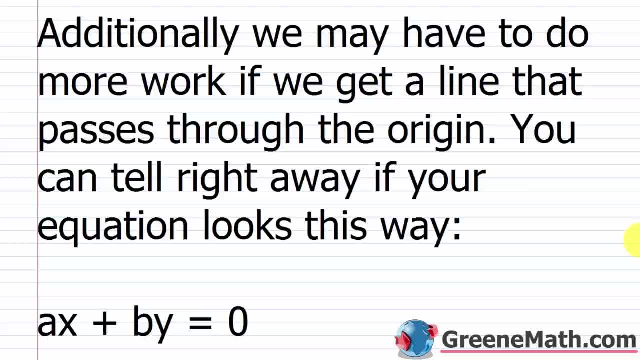 the previous two, But occasionally you're going to have to do a little bit more work because you're going to get a line that passes through the origin. You can tell right away if your equation looks like this: Ax plus by equals 0.. 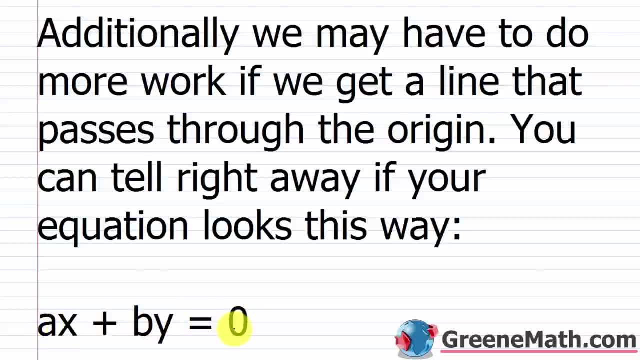 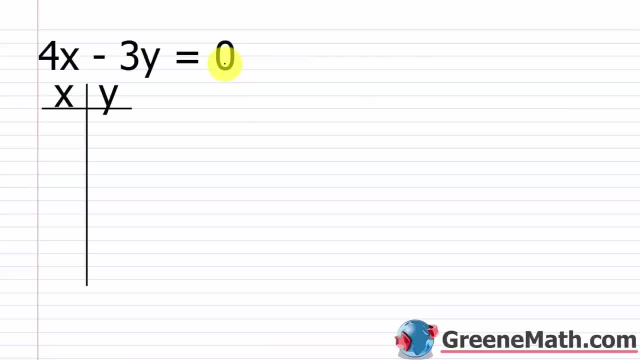 So some number times x plus some number times y equals 0. So we have an example here: x minus 3y equals 0. So the reason it's additional work is because if you try to use your intercept method here, the x and the y-intercept occur at the same point, which is 0 comma 0.. 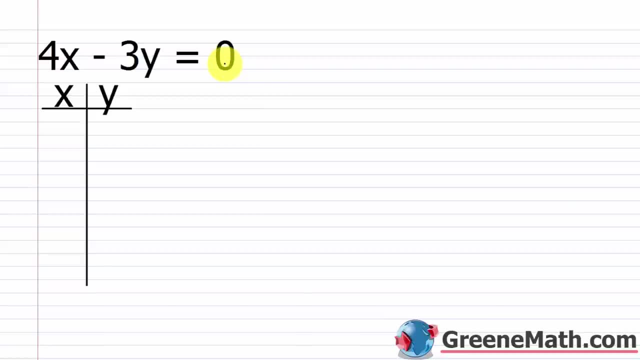 Right, The line passes through that, because that's the origin. If I plugged in a 0 for x- you can think about this term just going away- you'd have negative 3y equals 0.. Well, the only way negative 3y can equal 0 is if y is 0. 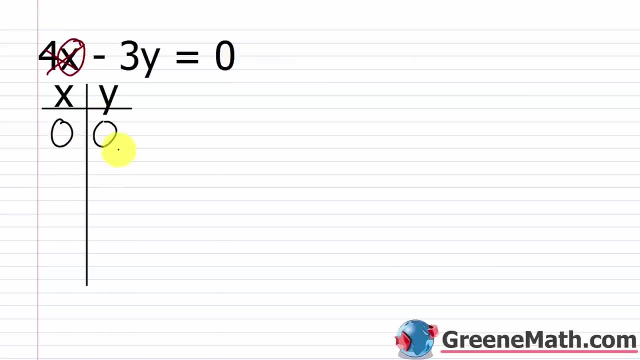 So 0 comma 0 is a point on that line. But now you can also see: okay, if y is 0,, x is 0, but x is 0y is also 0. So that's the only intercept I'm going to get. 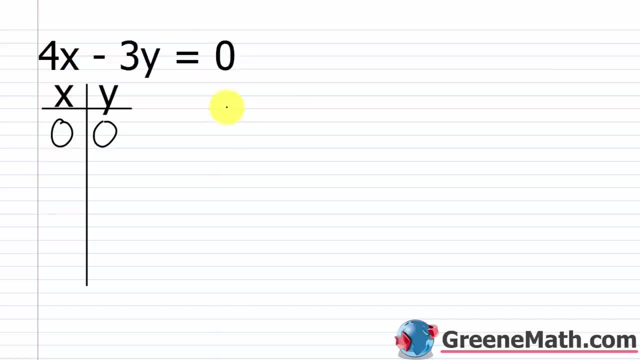 So now I have to pick 2 other points And I have: 4x minus 3y equals 0. So to make this a little easier myself, I'm just going to add 3y to both sides of the equation, And the reason I'm doing that is I want to make it a little easier to see. 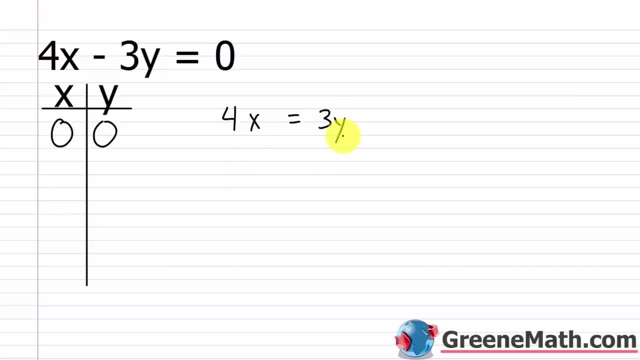 Okay, Okay, or choose something for y. the result of that is not going to be divisible by something to where I get an integer right. so in other words, if I plug in, let's say, a 3 here, I know that I'm going to get 12 and I know 12 is divisible by 3, so that will give me an integer so I can plug in a 3 here. 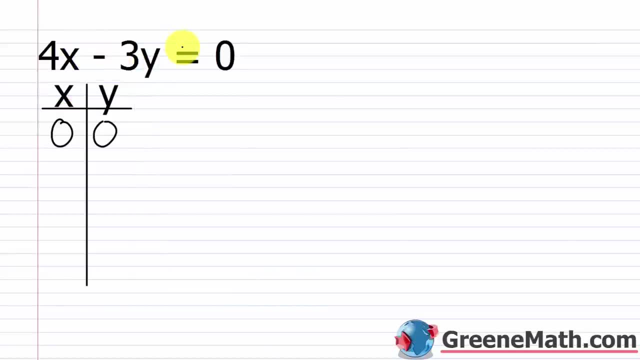 But now I can also see if y is 0, x is 0. But if x is 0, y is also 0. So that's the only intercepts I'm going to get. 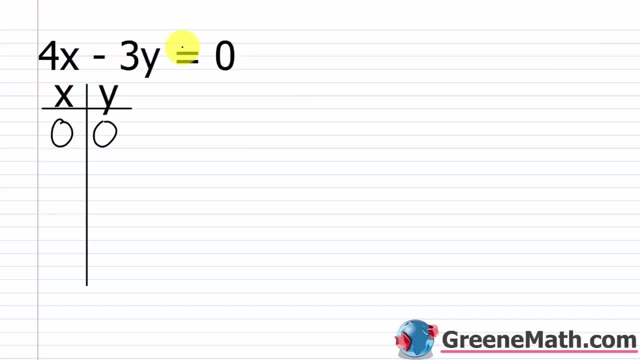 So now I have to pick two other points. And I have 4x minus 3y equals 0. 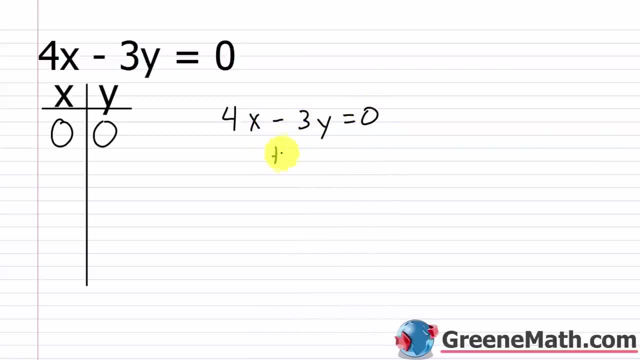 So to make this a little easy on myself, I'm just going to add 3y to both sides of the equation. 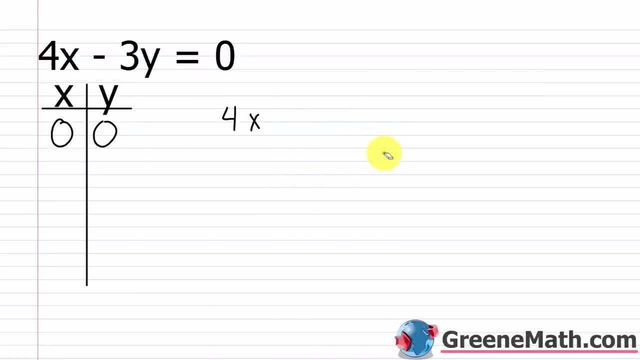 And the reason I'm doing that is I want to make it a little easier to see when I choose something for x or choose something for y, the result of that, is that going to be divisible by something to where I get an integer? In other words, if I plug in let's say a 3 here. I know that I'm going to get 12. 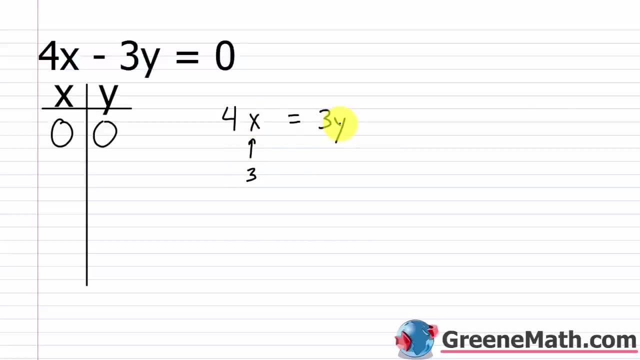 And I know 12 is divisible by 3. So that will give me an integer. So I can plug in a 3 here. And so this would be 12. 12 equals 3y, divide both sides by 3. And I get 4 is equal to y. make this really easy, 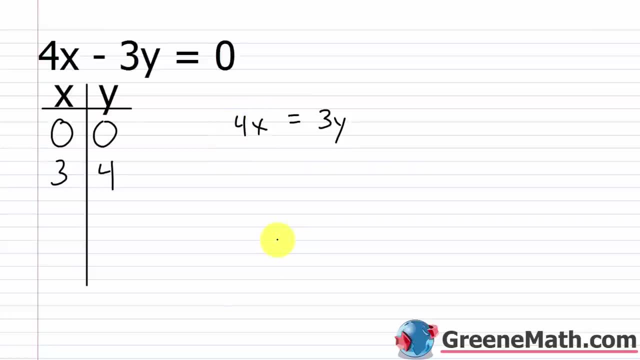 again I had 4x was equal to 3y, I could just use negative 3. 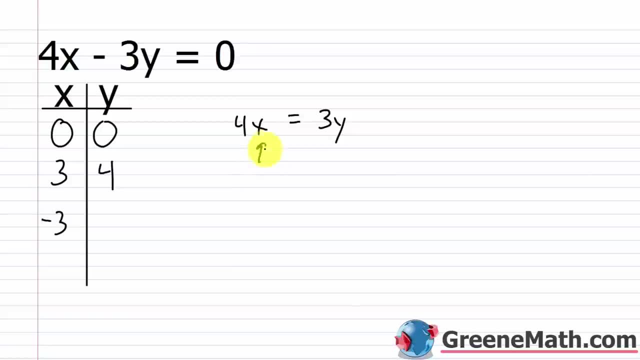 Because I know that's going to work out also. So what about negative 3 being plugged in for x. I'd have negative 12 equals 3y, divide both sides by 3. And I'll get negative 4 equals y. 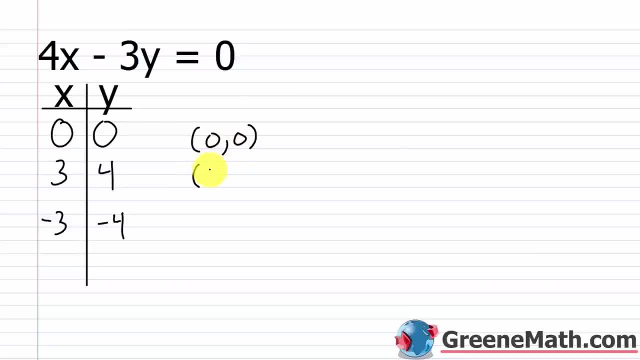 Alright, so I have my three ordered pairs. I have 0 comma 0. I have 3 comma 4. And I have negative 3 comma negative 4. 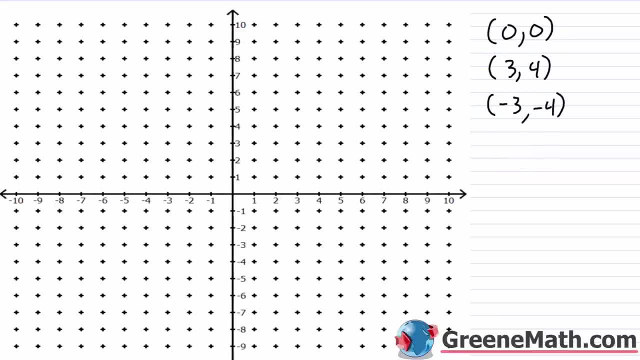 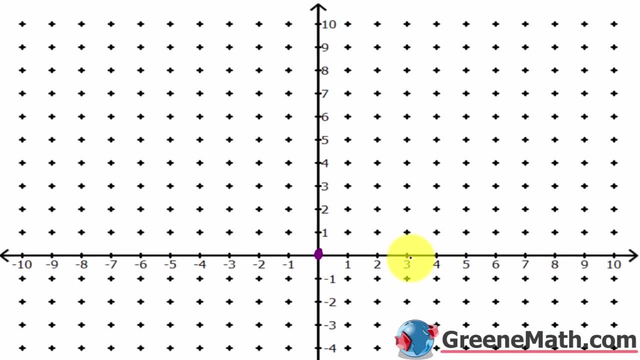 Okay, so let's plot these points. So 0 comma 0, that's at the origin. It's going to be right here. 3 comma 4. So go to the right 3, go up 4. That's right here. 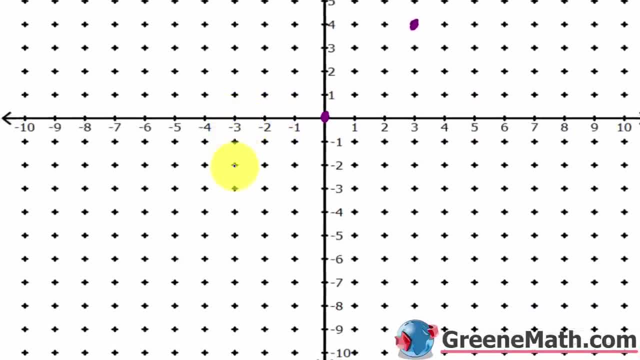 Negative 3 comma negative 4. So go to the left 3 and down 4. That's going to be right here. 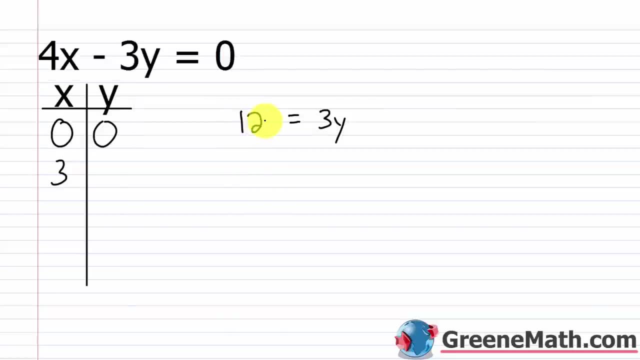 and so this would be 12. 12 equals 3y. divide both sides by 3 and I get 4 is equal to y. now, to make this really easy again, I had 4x was equal to 3y. I could just use negative 3, because I know that's going to work. 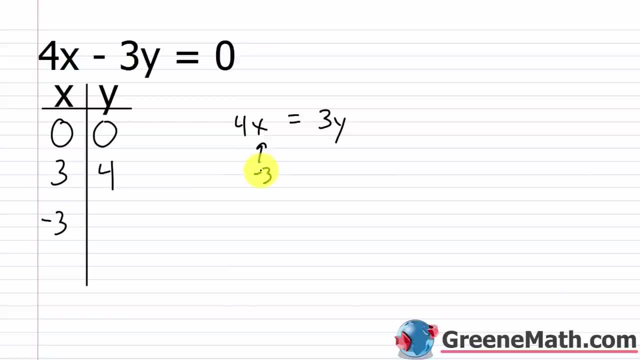 out also. so what about negative 3 being plugged in for x? I'd have negative 12 equals 3y. divide both sides by 3 and I'll get negative 4 equals y. all right, so I have my three ordered pairs. I have 0 comma 0, I have 3 comma 4 and I have 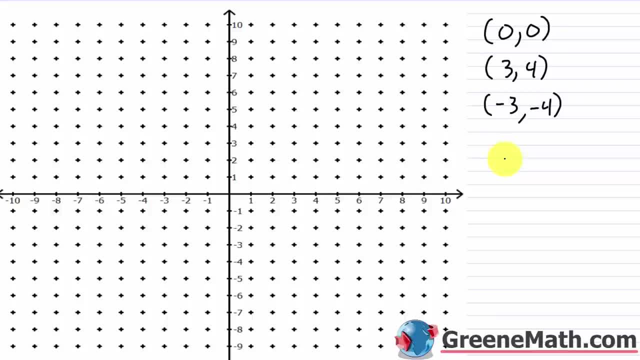 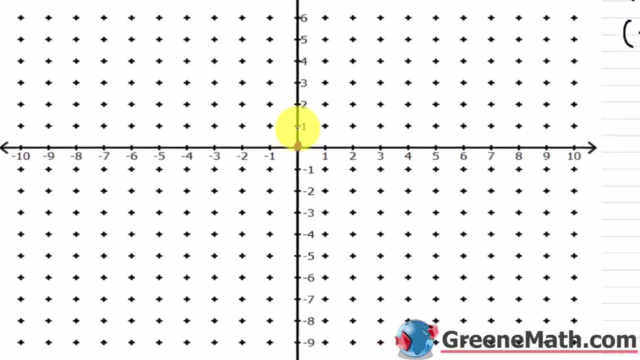 have negative 3 comma, negative 4.. Okay, so let's plot these points. So 0 comma 0, that's at the origin, that's going to be right here. 3 comma 4, so go to the right 3, go up 4, that's right here. 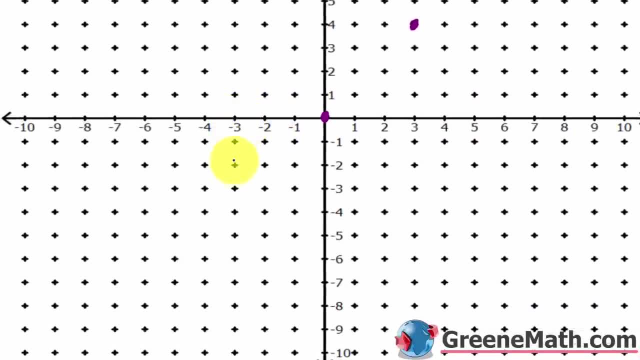 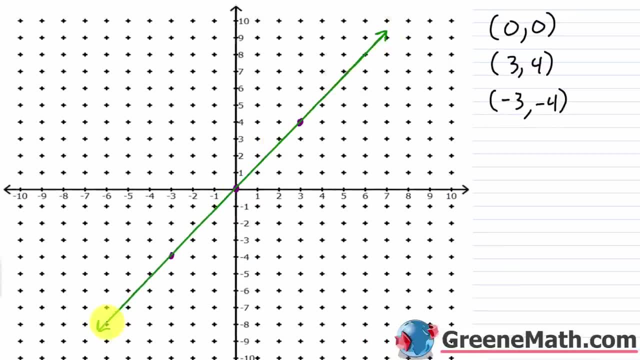 Negative 3, comma negative 4, so go to the left 3 and down 4, that's going to be right here. All right, we're going to put your arrows at each end And I'm going to go ahead and label this. 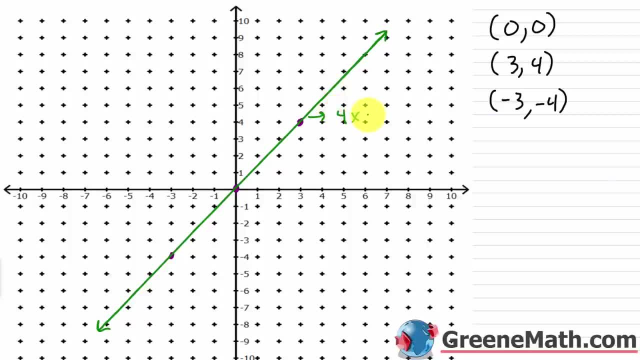 Again, this is the equation: 4x minus 3y equals 0. And you can see, the only place that this line crosses through the y-axis is at 0 comma 0. And the only place this line crosses through the x-axis is, again at 0 comma 0.. So this is a line through the origin where both the x-axis and 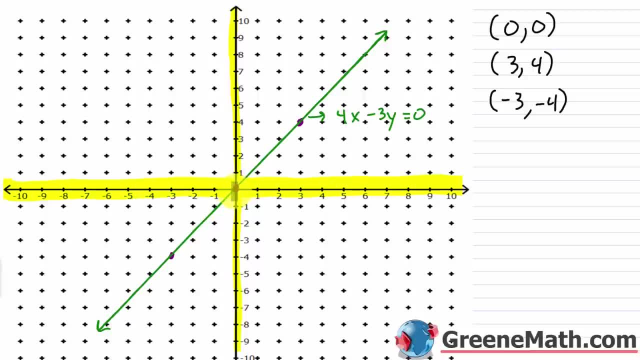 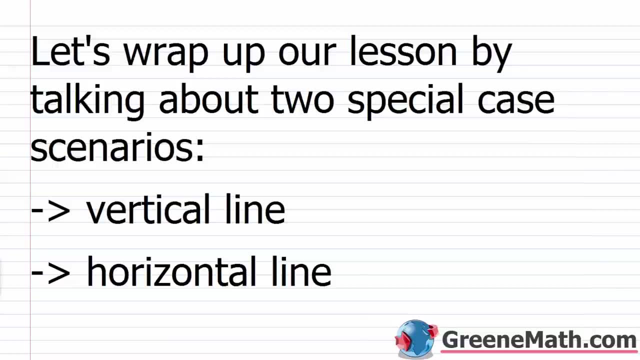 the y-axis cross and the y-intercept occur at that origin. 0 comma 0.. All right, so we've kind of talked about the basic scenarios that you're going to come across, And at this point you should be confident enough. 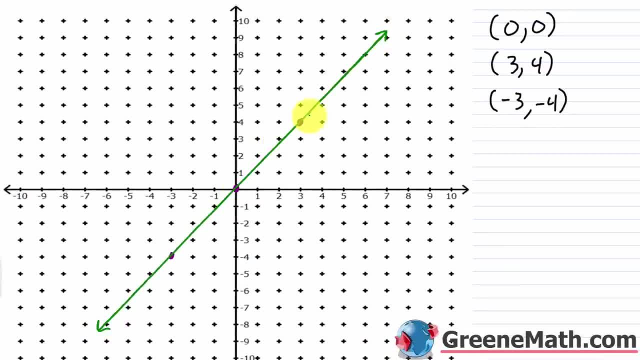 In order to put your arrows at each end. And I'm going to go ahead and label this. Again, this is the equation. 4x minus 3y equals 0. And you can see the only place that this line crosses through the y-axis is at 0 comma 0. 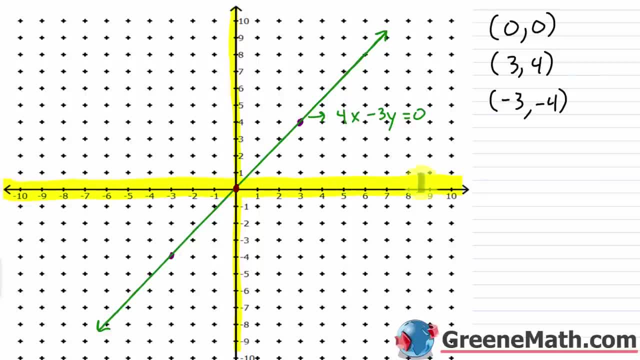 And the only place this line crosses through the x-axis is again at 0 comma 0. So this is a line through the origin, where both the x and the y-intercept occur at that origin, 0 comma 0. 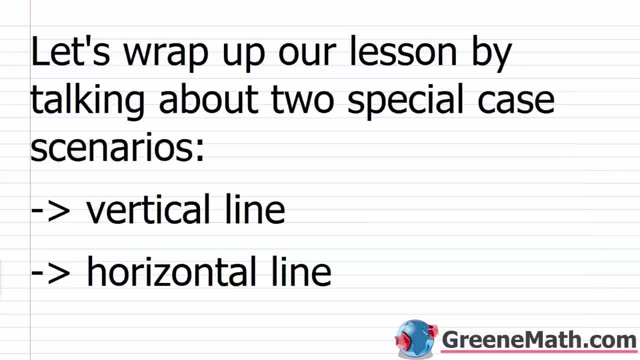 Alright, so we've kind of talked about the basic scenarios that you're going to come across. 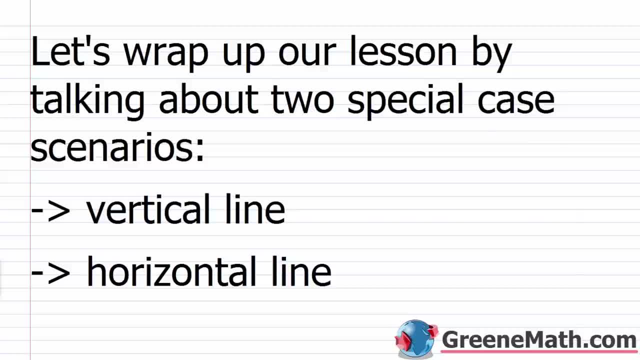 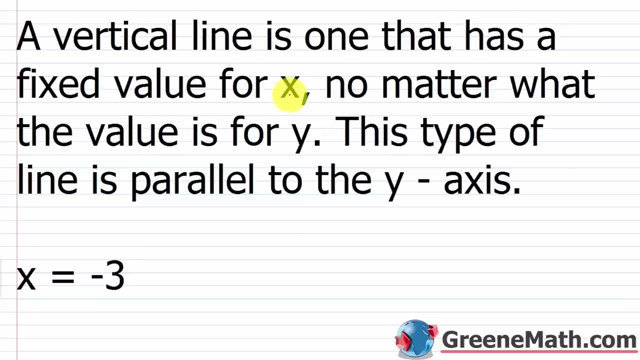 And at this point, you should be confident enough to be able to graph most of the linear equations in two variables that you're going to encounter. It's just something you need to practice at this point. But I want to wrap up our lesson by talking about two special case scenarios. And if you see these, you're going to kind of be confused about what to do. So the first one is a vertical line, and the second one is a horizontal line. So a vertical line is one that has a fixed value for x, no matter what the value is for y. 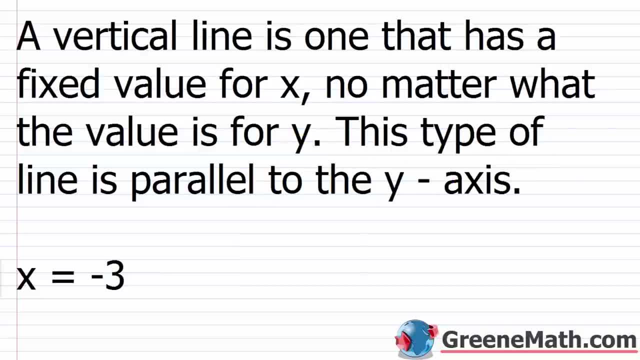 So this type of line is parallel to the y-axis. 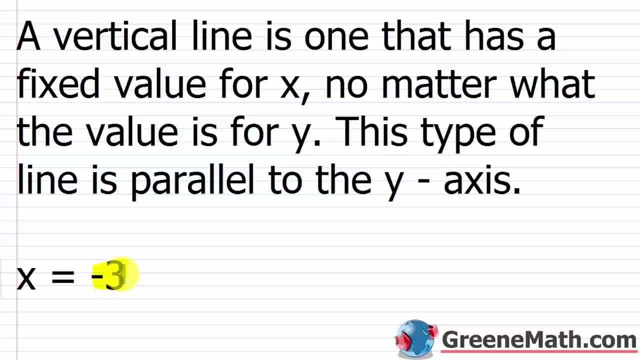 So we have x equals negative 3. So what we're saying here is that no matter what the value is for y, x is equal to negative 3. So if you want, 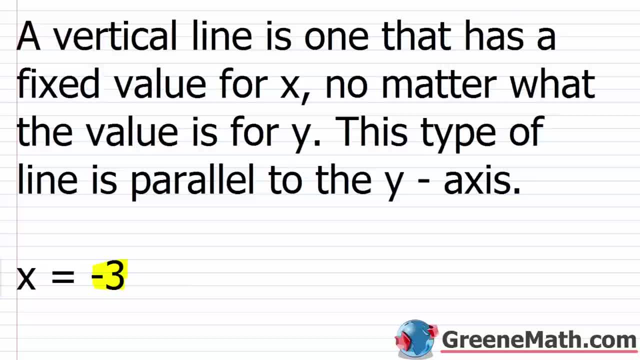 you can choose points and plot those points and draw a line. 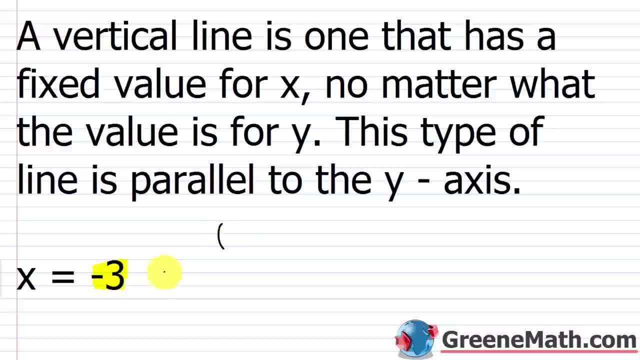 So in other words, I can pick some values for y, x is always negative 3, so I'd have negative 3 comma, I don't know, let's say negative 5. And then I could do negative 3 comma 0, and I could do negative 3 comma positive 5. No matter what I choose for y, it doesn't matter what it is, it could be 1 billion, x would be negative 3. So you can go through and plot these points like that. 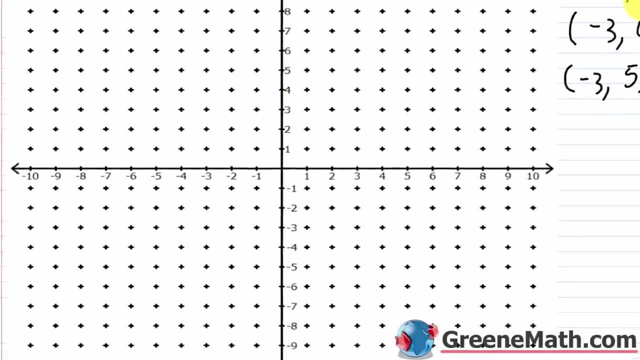 So we have negative 3 comma negative 5. So negative 3 negative 5, that's right here. Let me use a different color. And then negative 3 comma 0, that's right here. 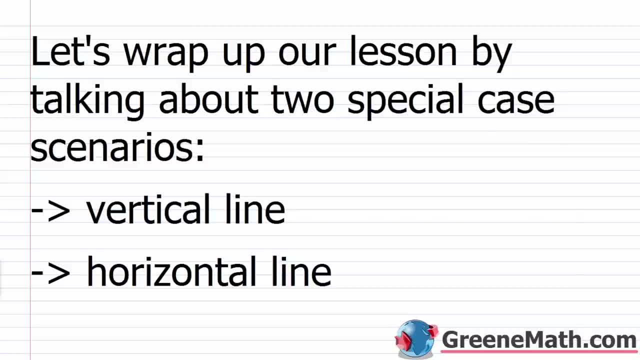 to be able to graph most of the linear equations in two variables that you're going to encounter. It's just something you need to practice at this point. But I want to wrap up our lesson by talking about two special case scenarios, And if you see these, you're going to kind of be confused about. 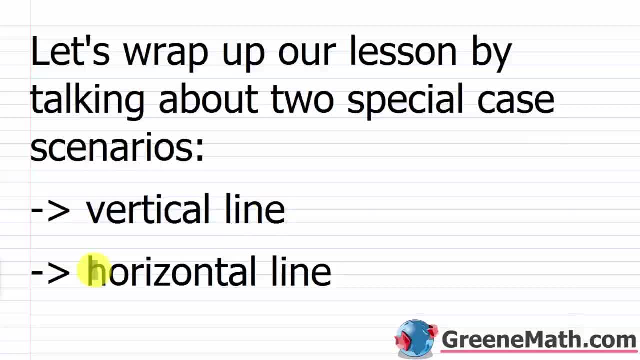 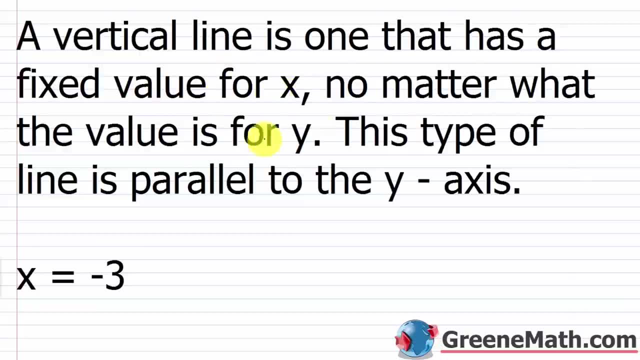 what to do. So the first one is a vertical line and the second one is a horizontal line. So a vertical line is one that has a fixed value for x, no matter what the value is for y. So this type of line is parallel to the y-axis. So we have x equals negative 3.. 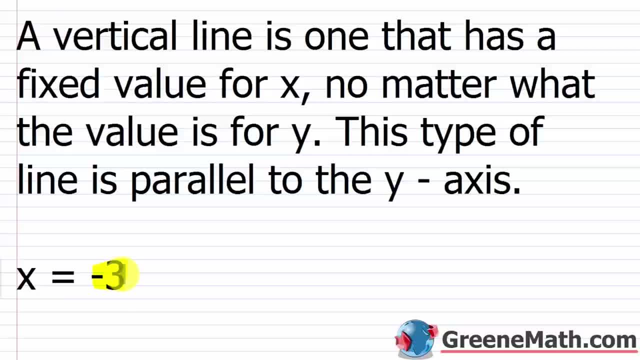 So what we're saying here is that, no matter what the value is for y, x is equal to negative 3.. So if you want, you can choose points and plot those points and draw a line. so in other words, I can pick some values for y, x is always negative 3, so I'd have negative 3,. 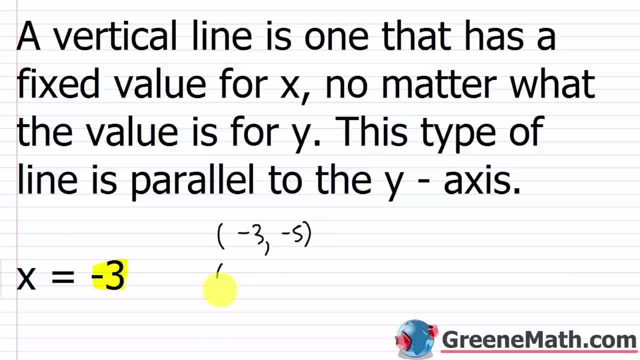 comma, I don't know. let's say negative 5. And then I could do negative 3, comma 0. And I could do negative 3, comma, positive 5. No matter what I choose for y, it doesn't matter. 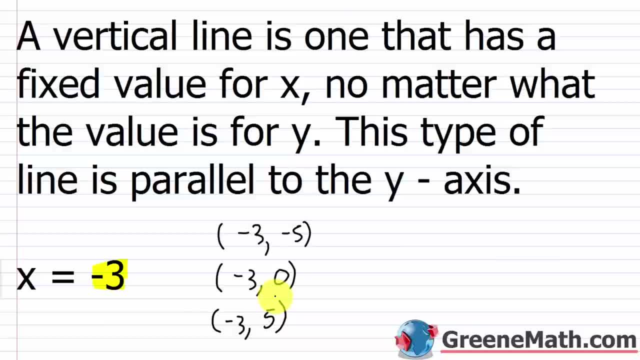 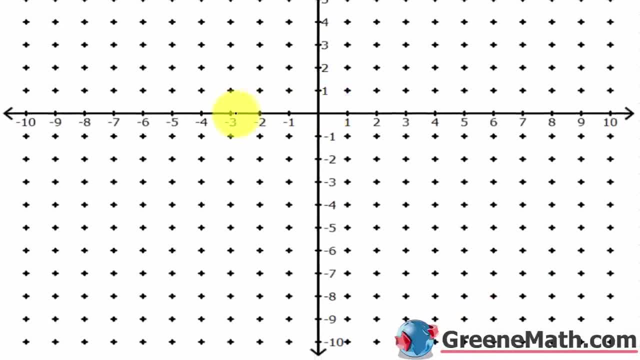 what it is. it could be 1 billion. x would be negative 3.. So you can go through and plot these points like that. So we have negative 3, comma negative 5.. So negative 3,, negative 5, that's right here. 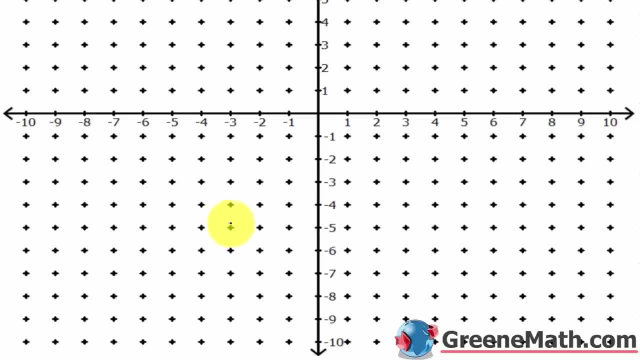 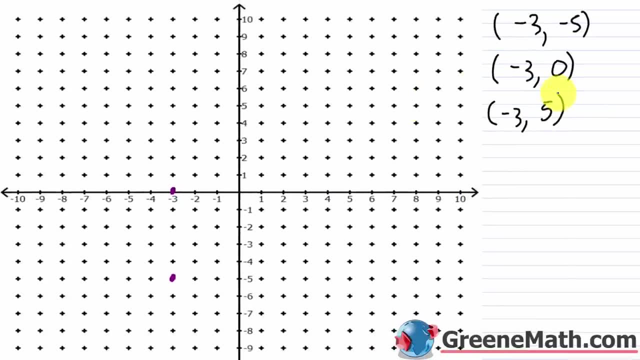 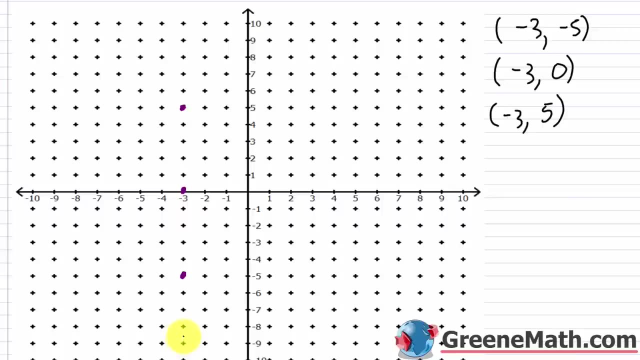 Let me use a different color, And then negative 3, comma 0, that's right here. And then negative 3, comma positive 5.. So that's going to be right here. So you can see you're going straight up and down, right. This would be a vertical line. 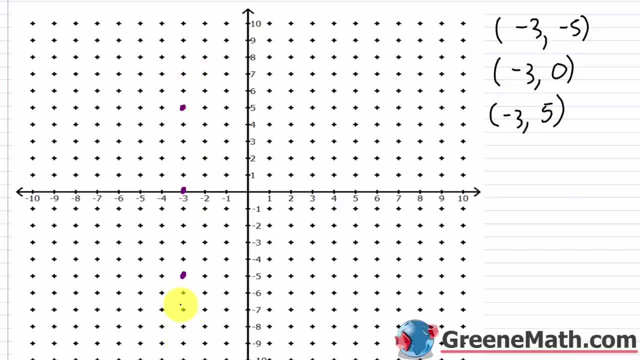 So the trick to this is, I don't need to make any points, You just kind of do that at first to get your mind wrapped around what's going on. If you have x equals negative 5, you just find negative 3 on the x-axis and you just create a vertical line. 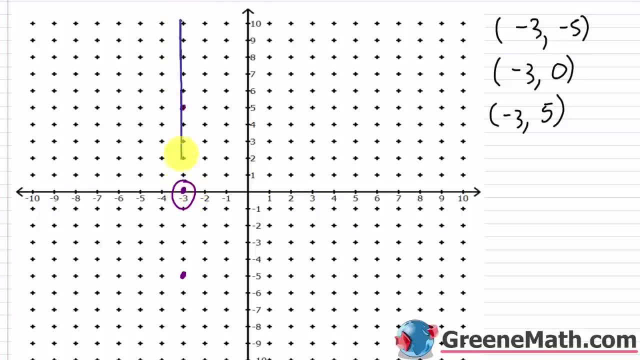 That's all you need to do. So I know that's not perfectly straight, but we'll just pretend that it is And we'll put our arrows at each end. And it's just that easy. And remember, no matter what the value of y is, let's say y is 7, x would be negative 3.. So this would be a. 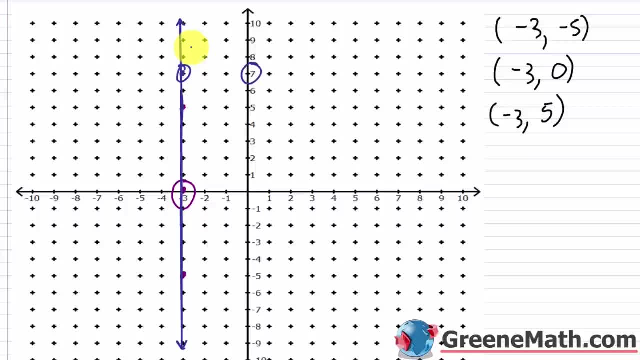 point on that line- And I know the line is kind of a little crooked, but it's not a point on that line, So it doesn't hit there, but that's where it should be. Or let's say y was negative 6. Well, x is negative 3.. So it's right there. 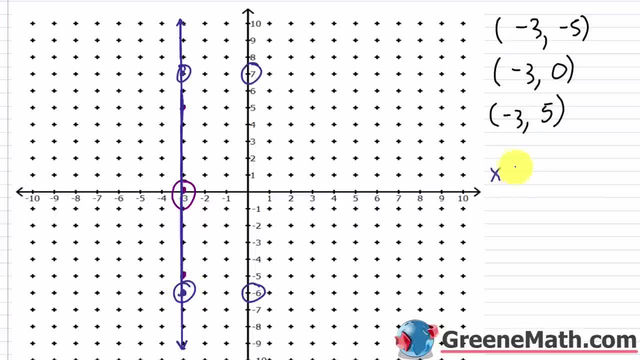 So if I gave you another one- let's say I gave you the problem- x is equal to positive 6.. Well, you just find 6 on the x-axis and you draw a vertical line. That's all you need to do. 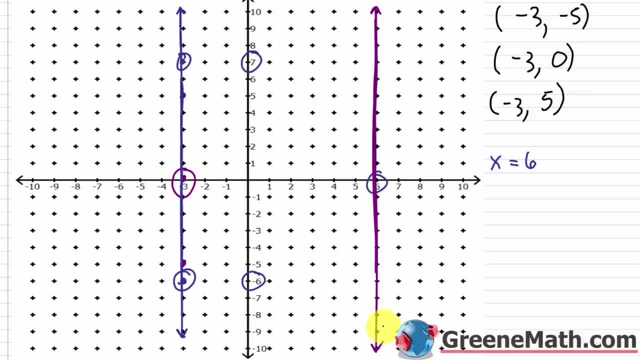 Okay, and again, I know that's not straight, but Do the best that I can. So put my arrows at each end. and that's: x equals 6.. So no matter what the value is for y, x will be 6.. So it's just a vertical line. 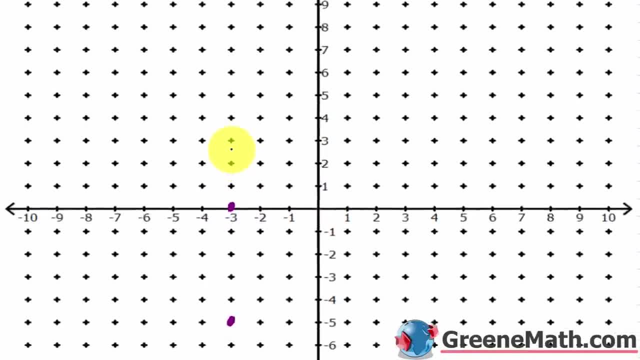 And then negative 3 comma positive 5, so that's going to be right here. So you can 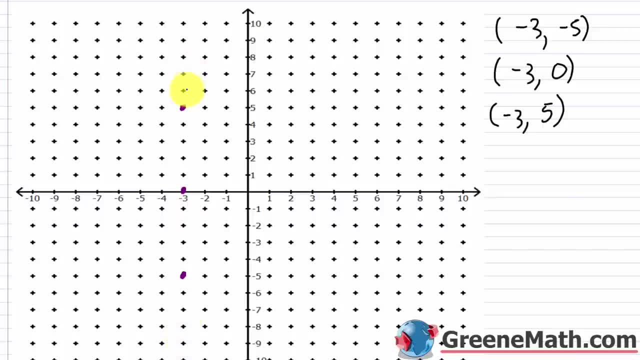 see you're going straight up and down. This would be a vertical line. So the trick to this is I don't need to make any points. 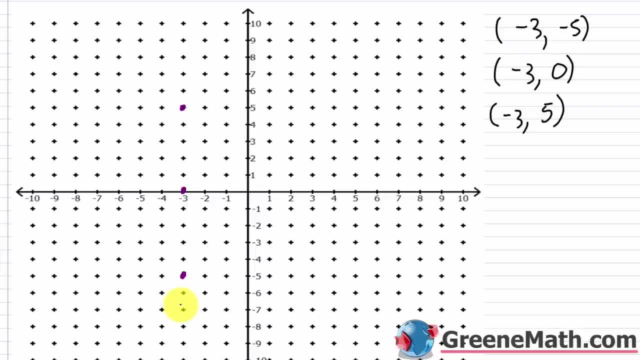 You just kind of do that at first to get your mind wrapped around what's going on. If you have x equals negative 3, you just find negative 3 on the x-axis, and you just create a vertical line. That's all you need to do. 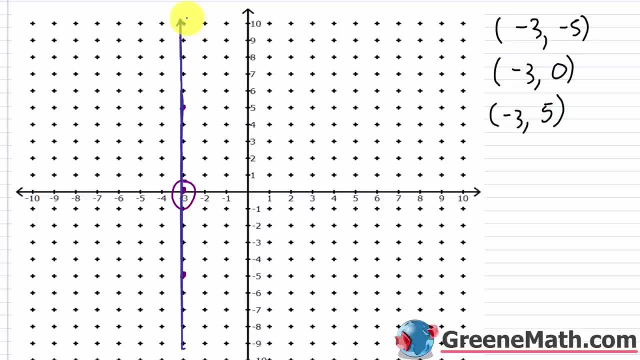 So I know that's not perfectly straight, but we'll just pretend that it is. 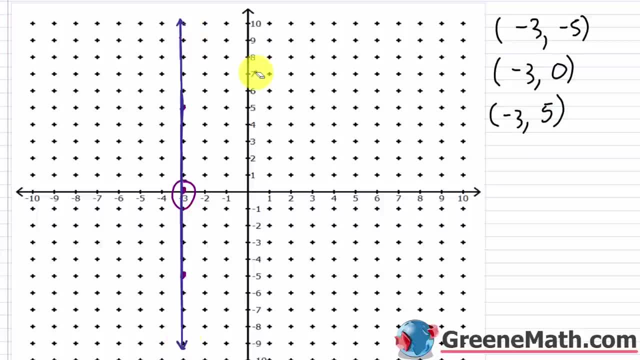 And we'll put our arrows at each end. And it's just that easy. 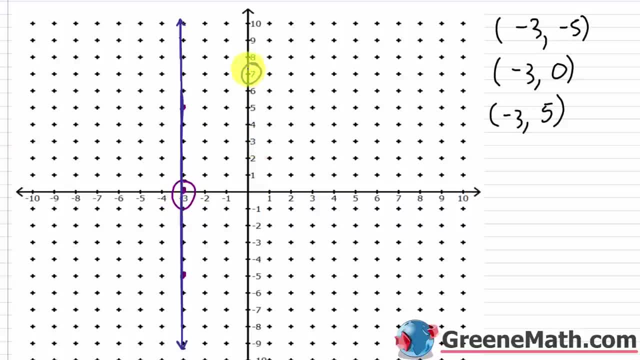 And remember, no matter what the value of y is, let's say y is 7, x would be negative 3. So this would be a point on that line. 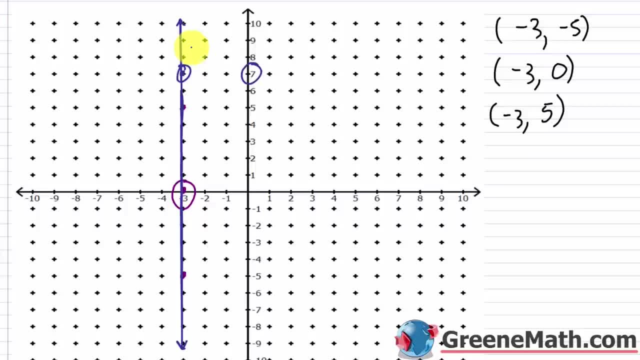 And I know the line is kind of a little crooked so it doesn't hit there, but that's where it should be. 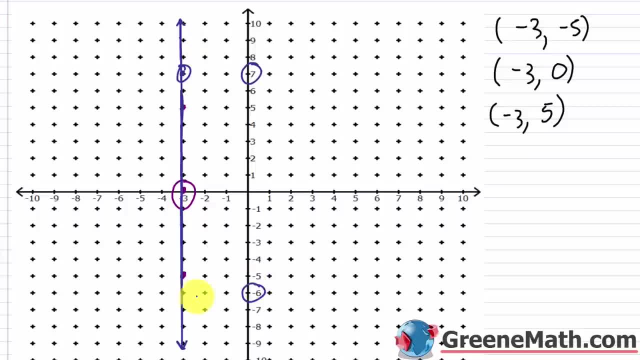 Or let's say y was negative 6. Well, x is negative 3. 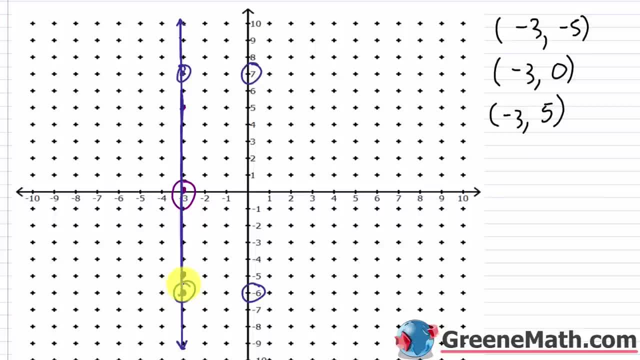 So it's right there. So if I gave you another one, let's say I gave you the problem x is equal to positive 6. Well, you just find 6 on the x-axis, and you draw a vertical line. That's all you need to do. ... ... 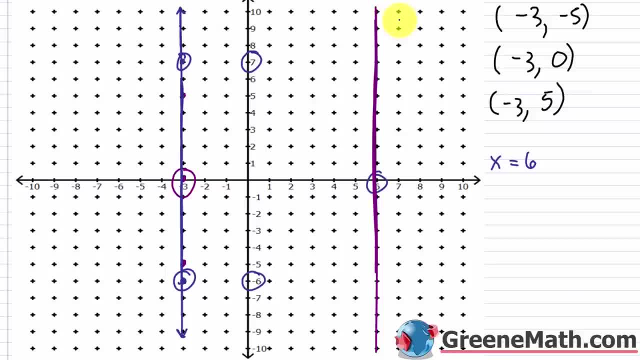 ... Okay, and again, I know that's not straight, 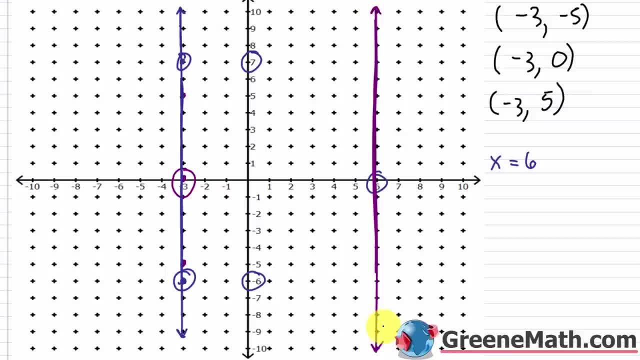 but I'll do the best that I can. So I put my arrows at each end, and that's x equals 6. So no matter what the value is for y, 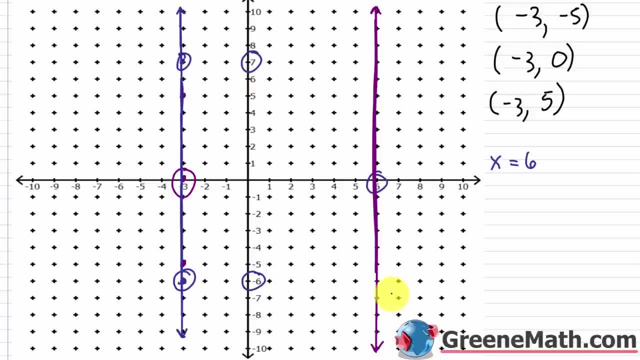 x will be 6. So it's just a vertical line. 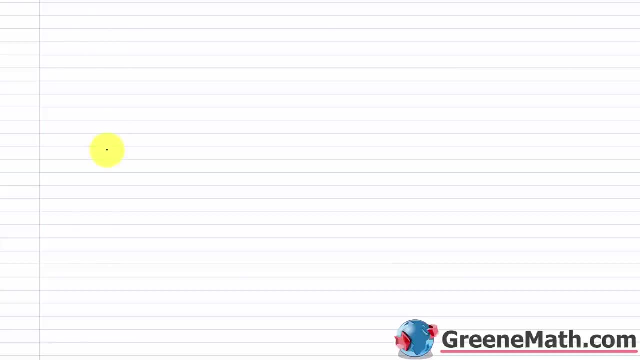 Now mathematically, you might be asking, how is this a linear equation in two variables? Well, let's go back to the definition I gave you when we first started talking about it. 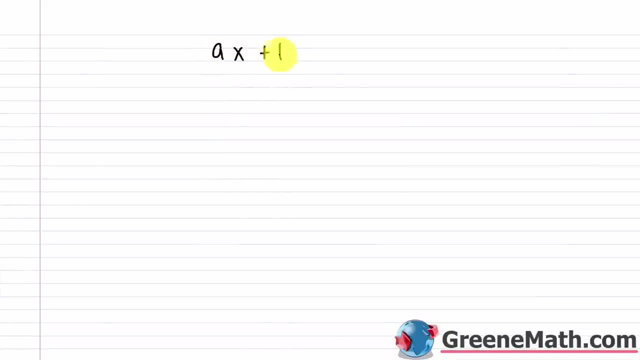 I said that we had ax, plus by, equals c, where ab and c were real numbers, and a and b were not both 0. 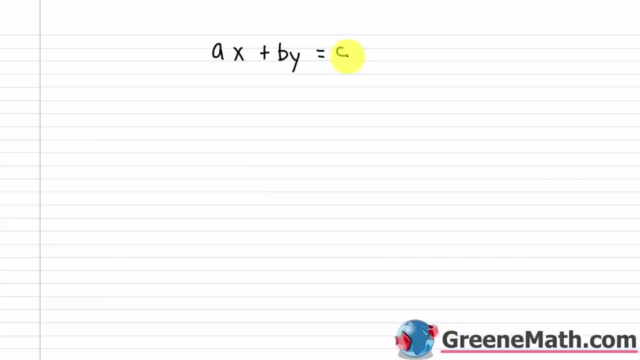 So, a and b are not both 0, but one of them could be. 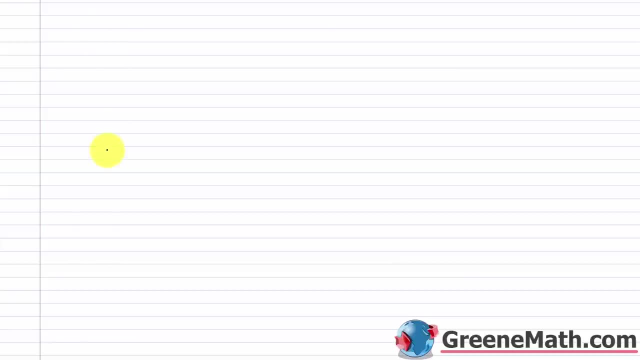 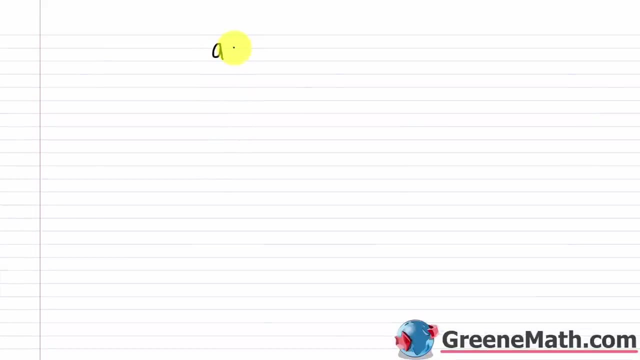 Now, mathematically, you might be asking: how is this a linear equation in two variables? Let's go back to the definition I gave you when we first started talking about it. I said that we had ax plus by equals c, where ab and c were real numbers and a and b were not both 0. 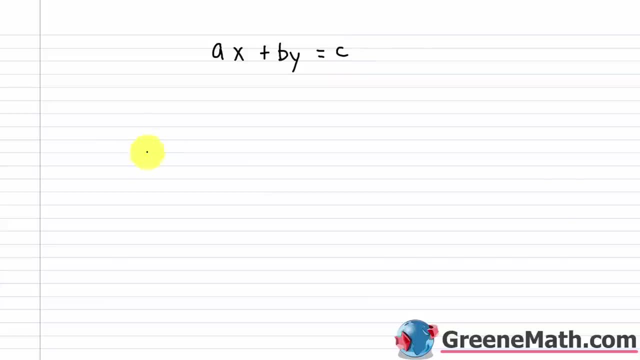 So a and b are not both 0, but one of them could be. So if I have 1x plus 0y equals some number, let's say negative 3, for example. When I simplify this I end up with 1x, or just x plus 0 times y is 0. 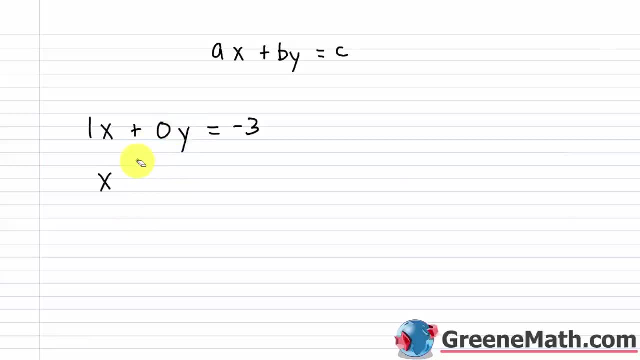 So I can just kind of get rid of that. So it'll really be x just equals negative 3.. So this is a way to write it as a linear equation in two variables, And it's also a way to write it as a linear equation in two variables. 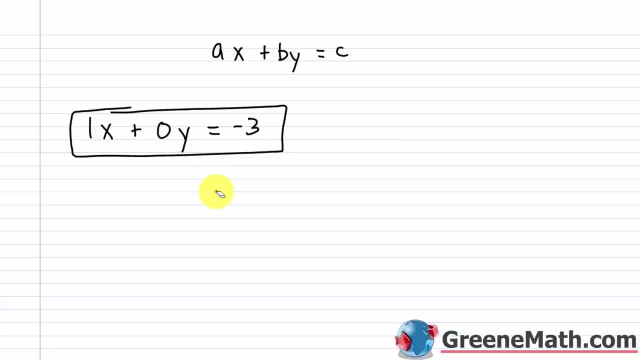 And it's also a way to check your ordered pairs right, to mathematically show that it makes sense. If I have the ordered pair negative 3 comma 5, well, I can plug it into this equation and it would be true. 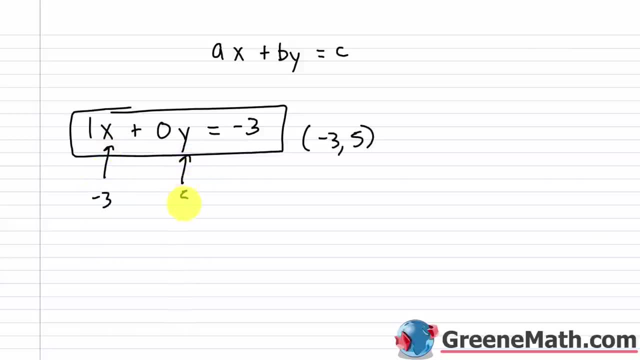 So I plug in a negative 3 for x and I plug in a 5 for y. 1 times negative 3 plus 0 times 5 should be equal to negative 3.. 1 times negative 3 is negative 3.. 0 times 5 is 0.. 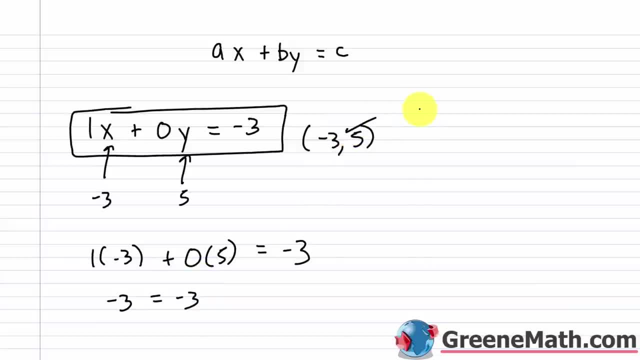 So this would be negative 3 equals negative 3.. So that checks out And you could do that As long as x is negative 3.. You could do that with any value of y, because you're multiplying it by 0, so it's just going to drop out. 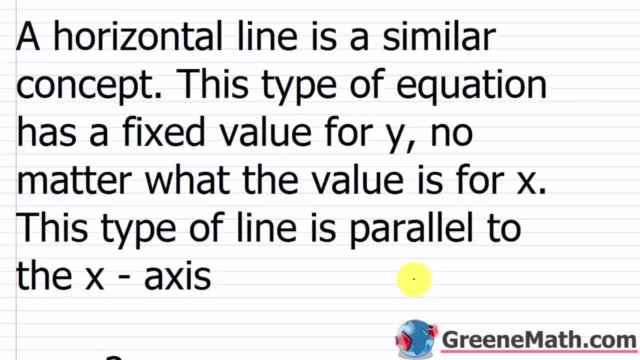 So the next concept is a horizontal line, And this is very, very similar to what we just looked at. This type of equation has a fixed value for y, no matter what the value is for x, So this type of line is going to be parallel to the x-axis. 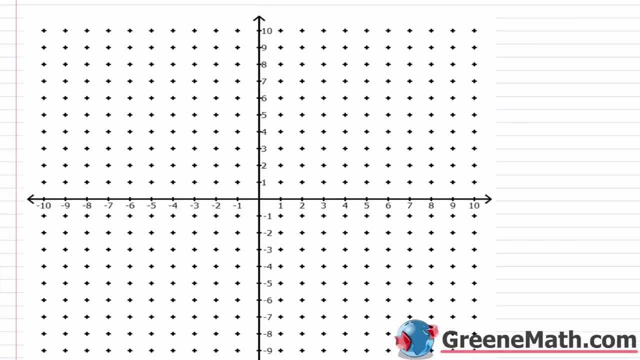 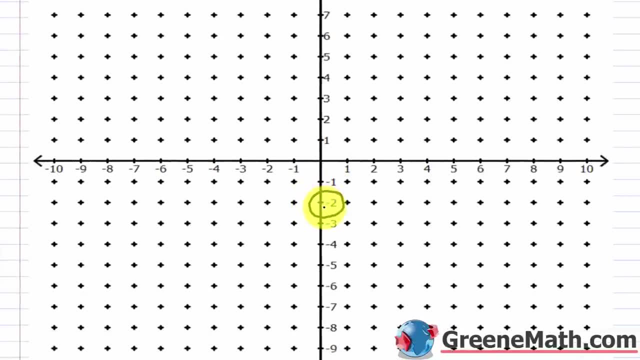 So let's look at: y equals negative 2, to start. And again, you could go through and make some points, but you don't need to If y equals negative 2.. Find negative 2 on the y-axis. It's right there. 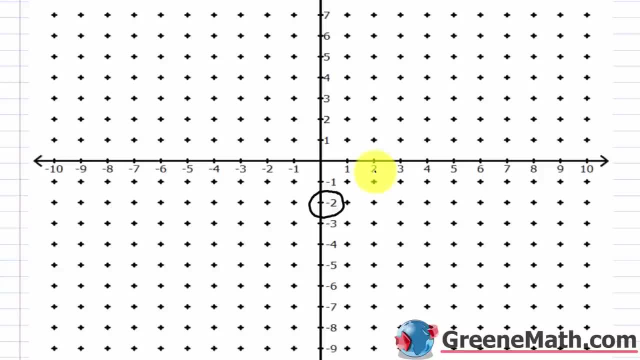 So no matter what the value is for x, let's say the value is 2 for x- y is negative. 2. Say the value is 6 for x, y is negative. 2. Say the value is 10 for x, y is negative 2.. 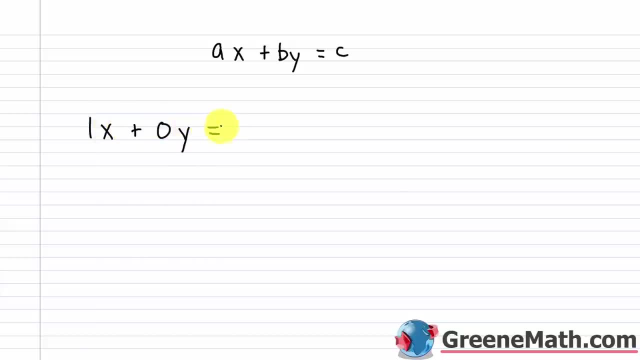 So if I have 1x plus 0y equals some number, let's say negative 3, for example, when I simplify this, I end up with 1x, or just x, plus 0 times y is 0, so I can just kind of get rid of it. 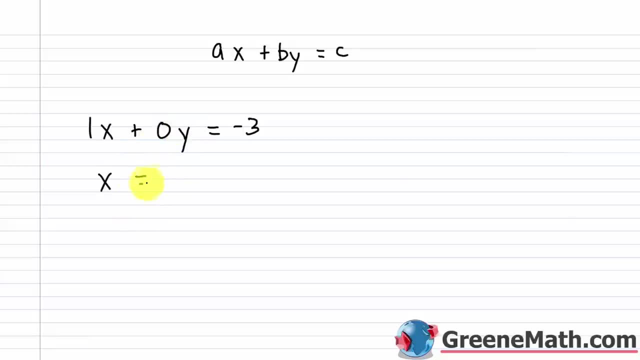 So it will really be x just equals negative 3. 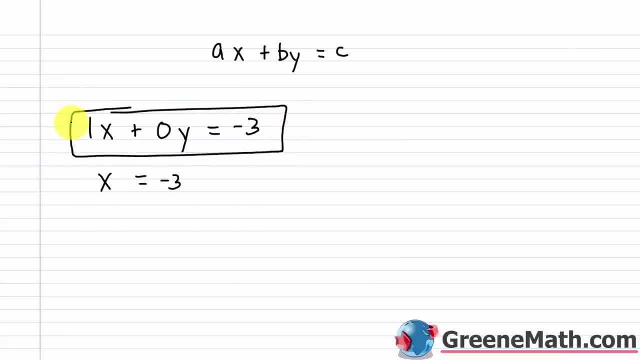 So this is a way to write it as a linear equation in two variables. 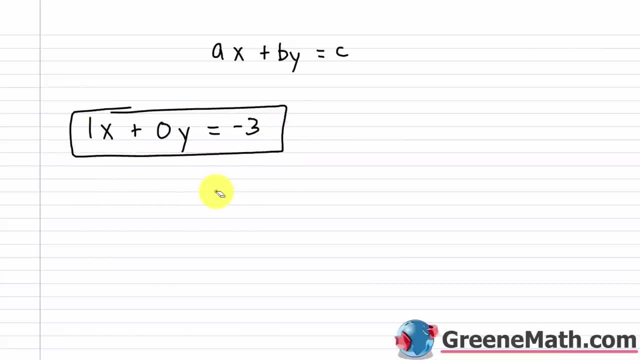 And it's also a way to check your ordered pairs, to mathematically show that it makes sense. 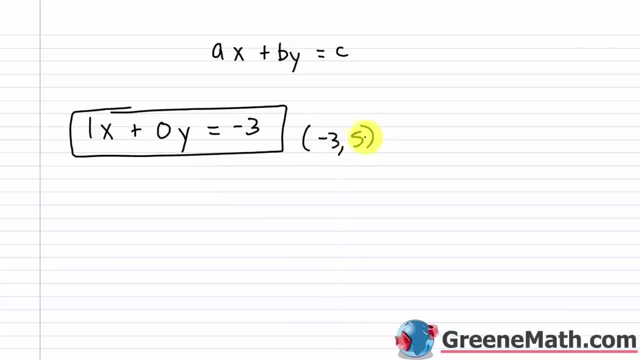 If I have the ordered pair, negative 3 comma 5, well I can plug it into this equation, and it would be true. 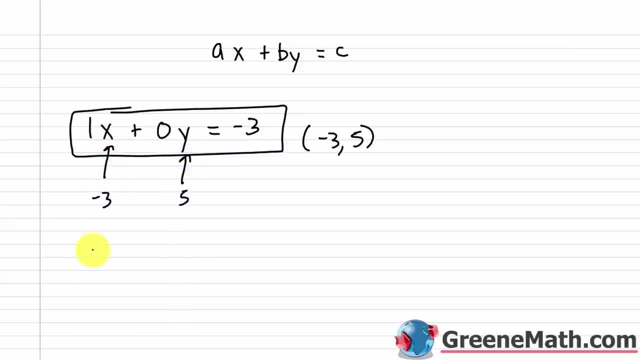 So I plug in a negative 3 for x, and I plug in a 5 for y. 1 times negative 3, plus 0 times 5, is 3. 1 times negative 3 is negative 3. 0 times 5 is 0, so this would be negative 3 equals negative 3. So that checks out. 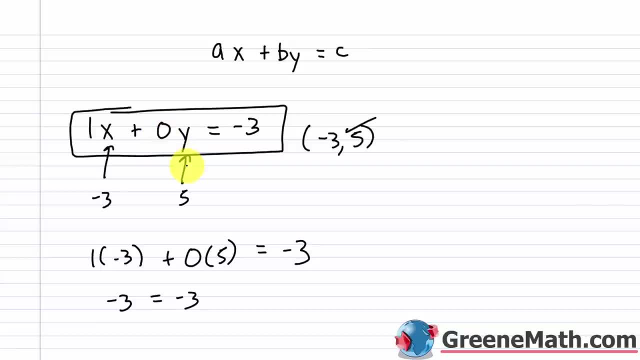 And you could do that, as long as x is negative 3, you could do that with any value of y, because you're multiplying it by 0, so it's just going to drop out. 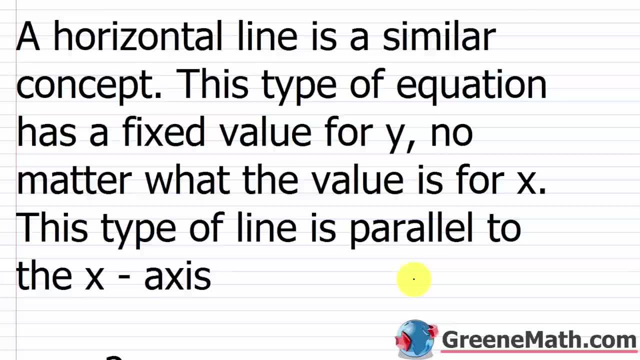 So the next concept is a horizontal line. And this is very, very similar to what we just looked at. This type of equation has a fixed value for y, and it should be parallel to the x-axis. 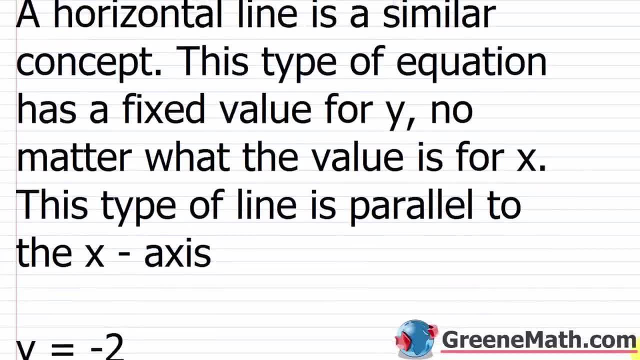 So let's look at y equals negative 2 to start. And again, you could go through and make some points, but you don't need to. 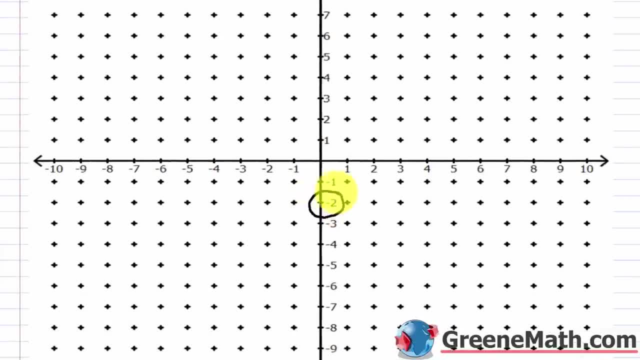 If y equals negative 2, find negative 2 on the y-axis. It's right there. 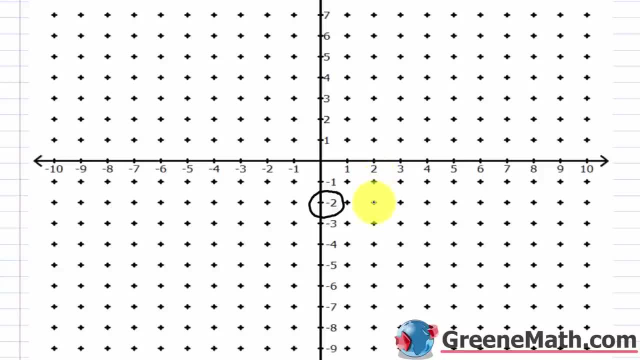 So no matter what the value is for x, let's say the value is 2 for x, y is negative 2. 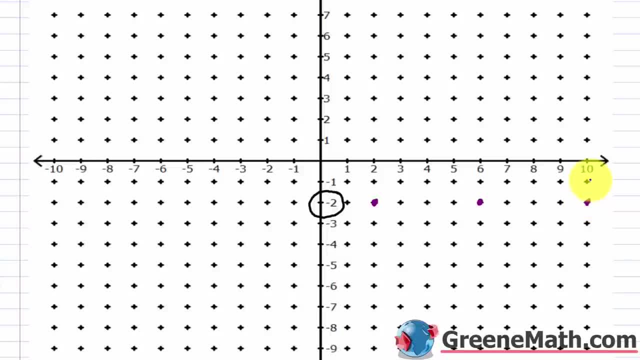 Say the value is 6 for x, y is negative 2. Say the value is 10 for x, 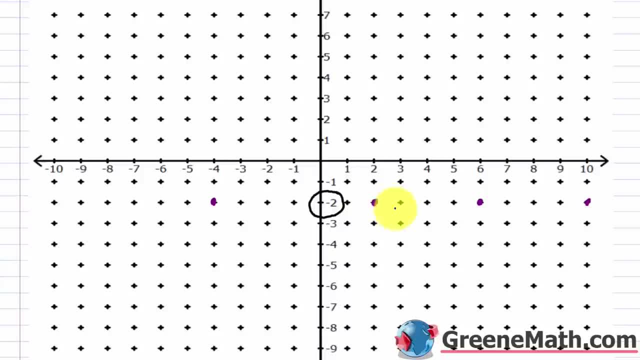 y is negative 2. So it's just a horizontal line. Just find negative 2 and draw a horizontal line. 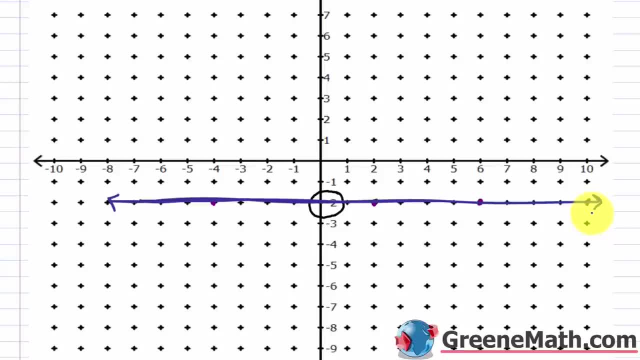 Alright, so that would be y equals negative 2. y equals negative 2. 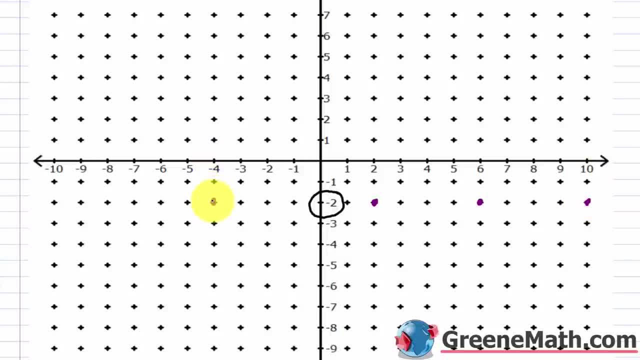 Say the value is negative 4 for x, y is negative 2.. So it's just a horizontal line. You just find negative 2 and draw a horizontal line. Okay, All right. so that would be: y equals negative 2,, y equals negative 2.. 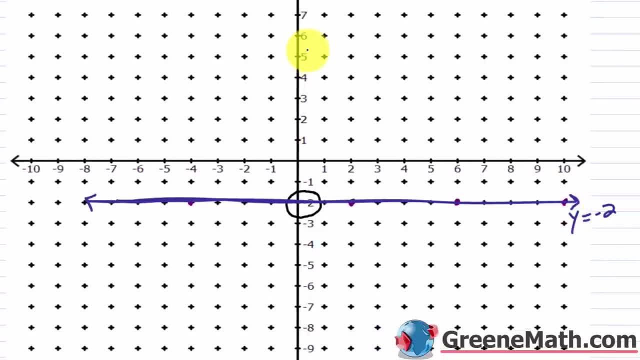 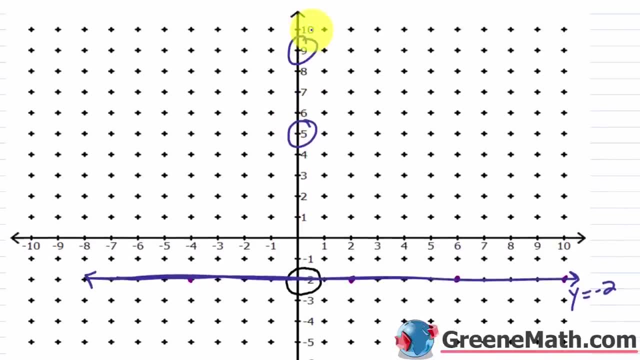 Now, if I said y equals 5,, I would just find 5 on the y-axis, draw a horizontal line. If I said y equals 9,, find 9 on the y-axis, draw a horizontal line. So these types of problems are very, very easy. 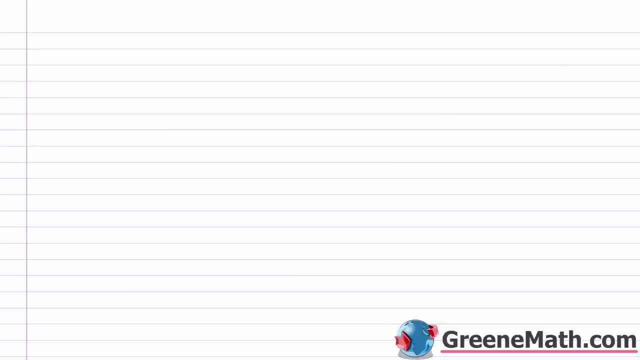 And again, mathematically we can write it as 0x plus 1y, So y equals. in that case it would be negative 2.. This is the same thing as y equals negative 2.. But we wrote it with two variables, so we can say it's a linear equation in two variables. 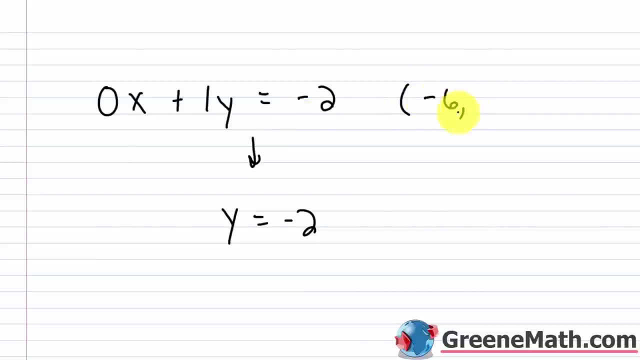 And if I give you an ordered pair like, let's say, negative 6 comma, negative 2, it's going to work. Plug in negative 6 for x: 0 times negative 6 is 0. So I'm just left with 1 times y. 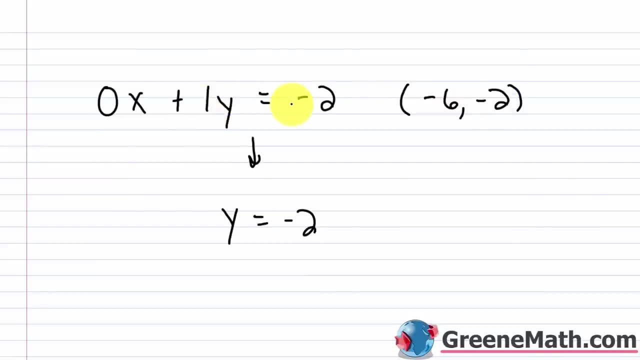 Plug in a negative 2 for y get negative 2 equals negative 2.. And so when you see an equation in this format, y equals some number. Find that number on the y-axis and draw a horizontal line. Hello and welcome to Algebra 1, Lesson 16.. 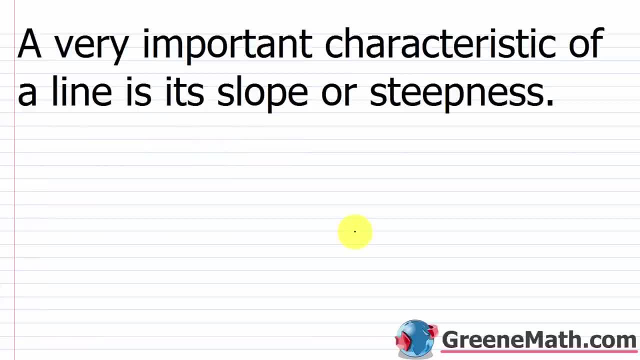 In this video we're going to learn how to find the slope of a line. So in our last lesson we learned how to graph a linear equation in two variables, Kind of. the next thing we want to learn how to do is take this graph right. 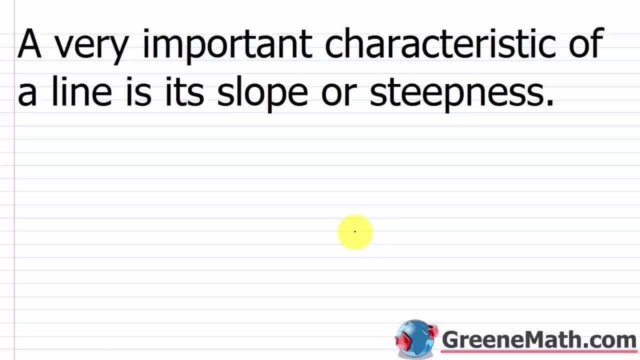 It's always of a line. That's why we call it a linear equation And analyze the steepness. right, The steepness is referred to as the slope. So I have here that a very important characteristic. A characteristic of a line is its slope. 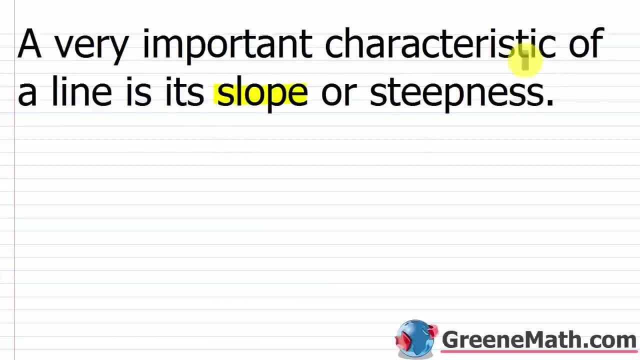 Let me highlight that word for you. It's slope or steepness, And you might not have run across this yet in your math class, but you've seen it in your everyday life. You can think about being on the interstate and seeing a 10% downgrade sign right. 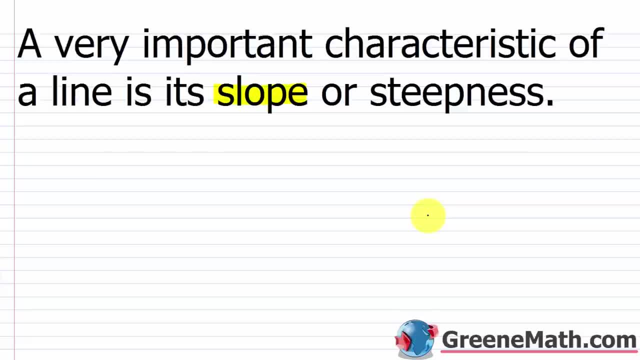 What does that mean? Well, it means, for every 10 miles you travel, the road has dropped by a mile. right, That's what a 10% downgrade means. Your road is going to look something like this: It's slanted. 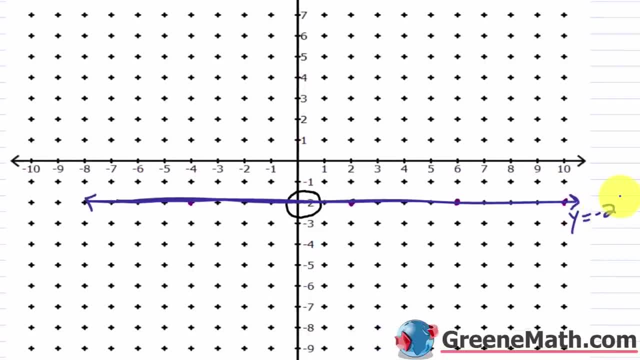 Now, if I said y equals 5, I would just find 5 on the y-axis, draw a horizontal line. 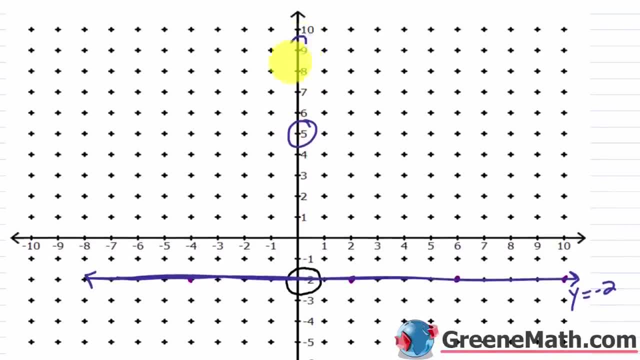 If I said y equals 9, find 9 on the y-axis, draw a horizontal line. So these types of problems are very, very easy. 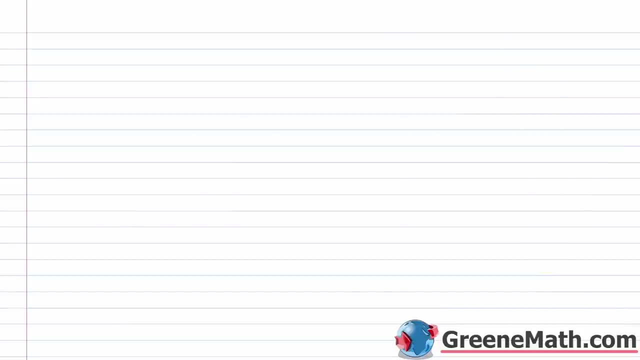 And again, mathematically, we can write it as 0x plus 1y equals, in that case it would be negative 2. 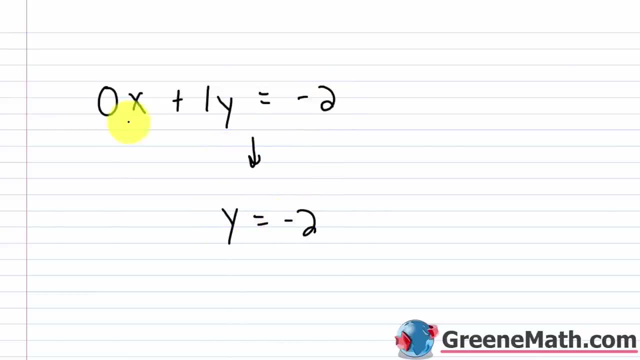 This is the same thing as y equals negative 2. But we wrote it with two variables, so we can say it's a linear equation in two variables. 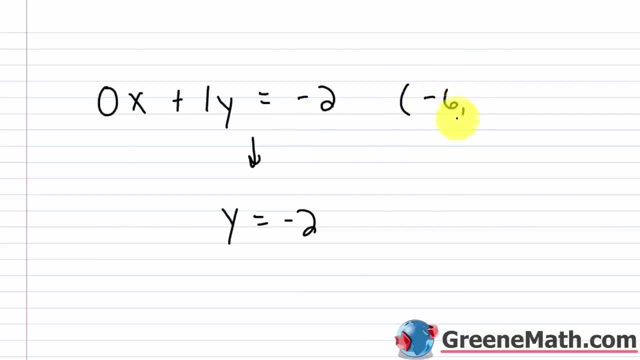 And if I give you an ordered pair, like let's say negative 6 comma negative 2, it's going to work. 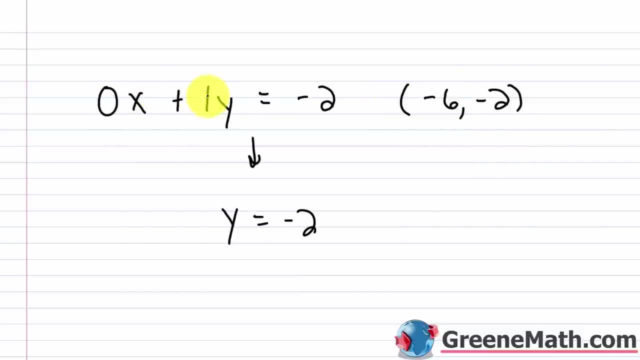 Plug in negative 6 for x, which times negative 6 is 0. 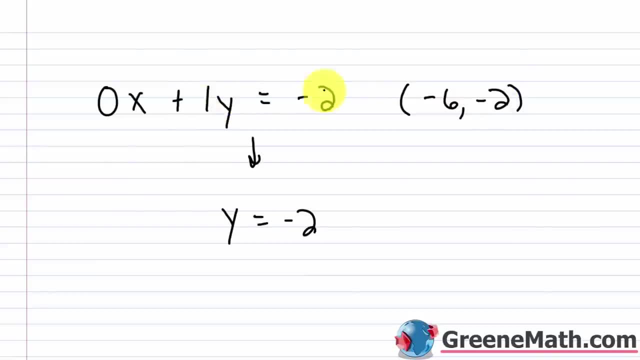 So I'm just left with 1 times y. Plug in a negative 2 for y, get negative 2 equals negative 2. And so, when you see an equation in this format, 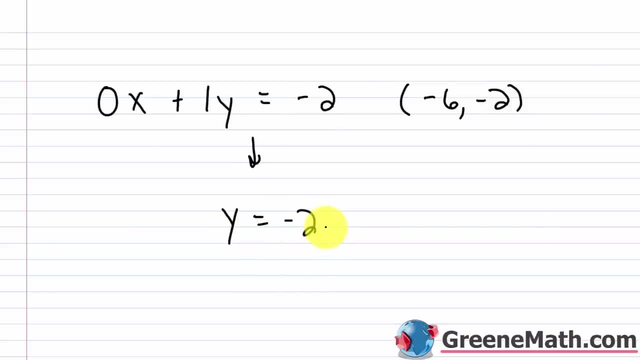 y equals some number. Find that number on the y-axis, and draw a horizontal line. Hello, and welcome to Algebra 1 Lesson 16. 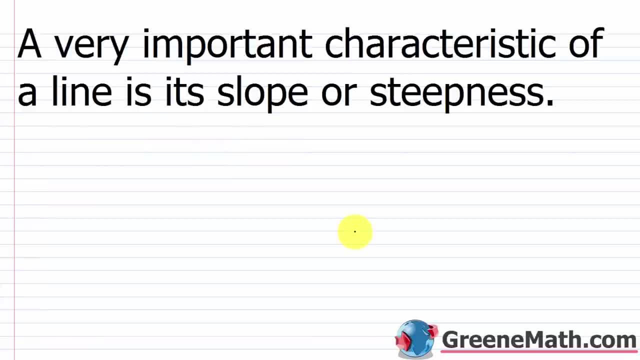 In this video, we're going to learn how to find the slope of a line. 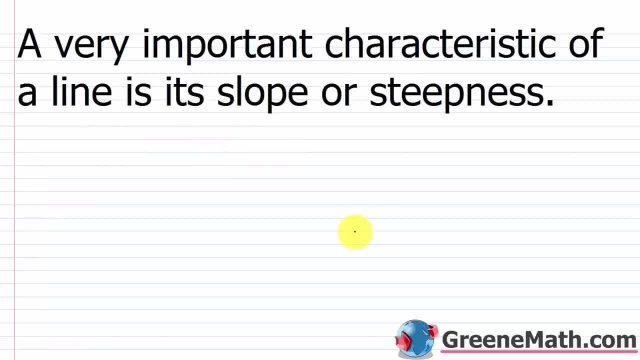 So in our last lesson, we learned how to graph a linear equation in two variables. Kind of the next thing we're going to learn how to do is 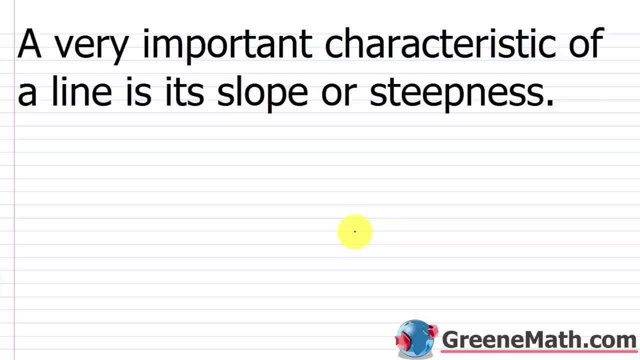 take this graph, it's always of a line, that's why we call it a linear equation, and analyze the steepness. 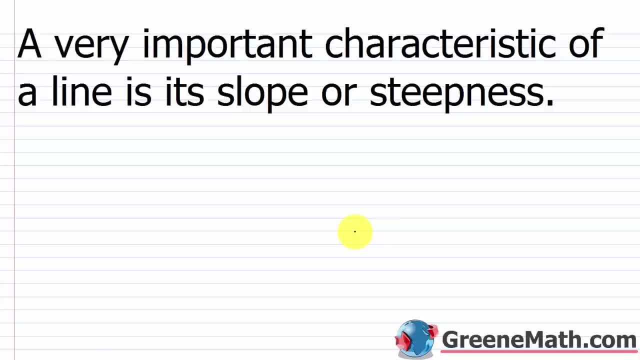 The steepness is referred to as the slope. 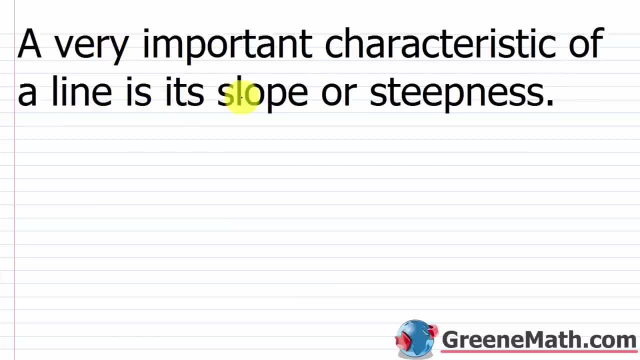 So I have here that a very important characteristic of a line is its slope, let me highlight that word for you, its slope, or steepness. 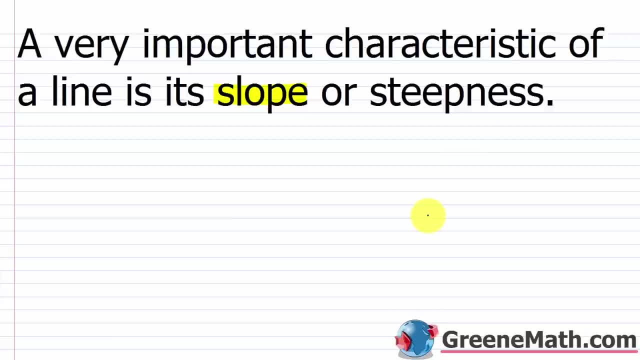 And you might not have run across this yet in your math class, but you've seen it in your everyday life. 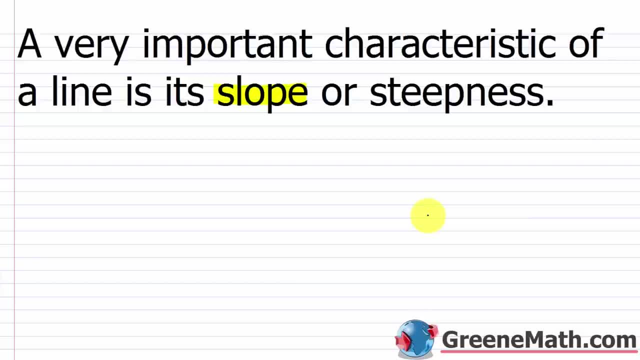 You can think about being on the interstate and seeing a 10% down grade sign. 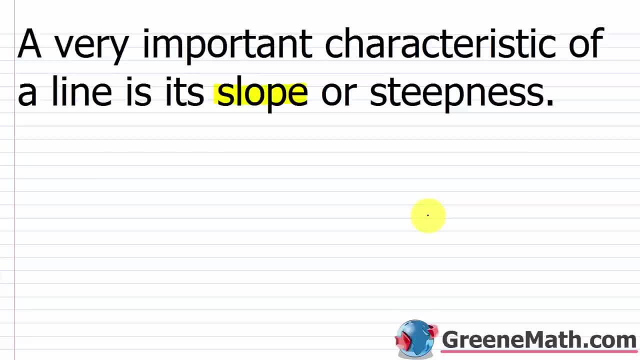 What does that mean? Well, it means for every 10 miles you travel, the road has dropped by a mile. That's what a 10% down grade means. 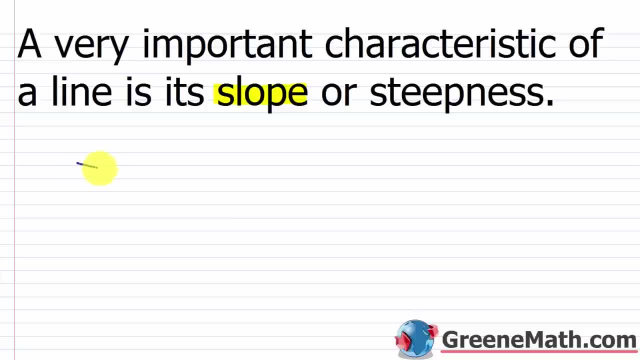 Your road is going to look something like this. It's slanted downward. I know that's not a perfectly straight line, but let me draw a picture of a little car here. 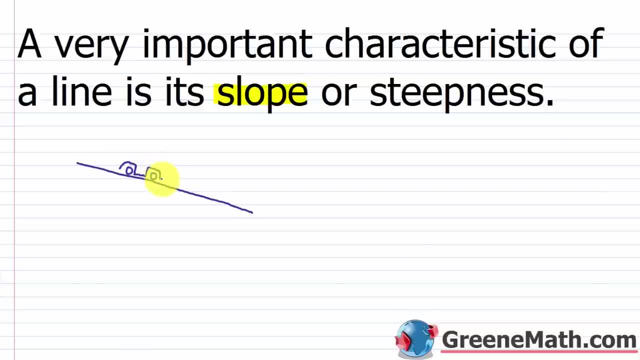 And just for the record, I am a terrible drawer, and I know that. So this is my car here. 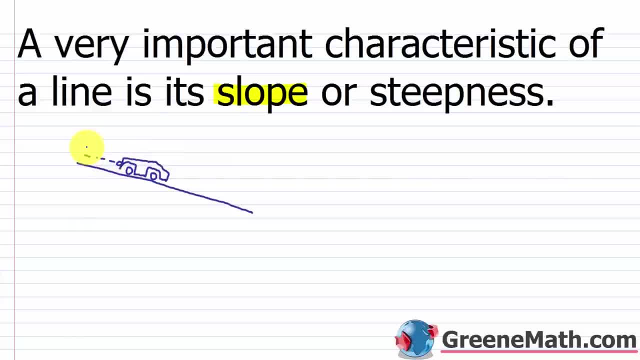 And I put a little exhaust going out of there. And I'm driving, and for every 10 miles I go, the road is dropping by a mile. 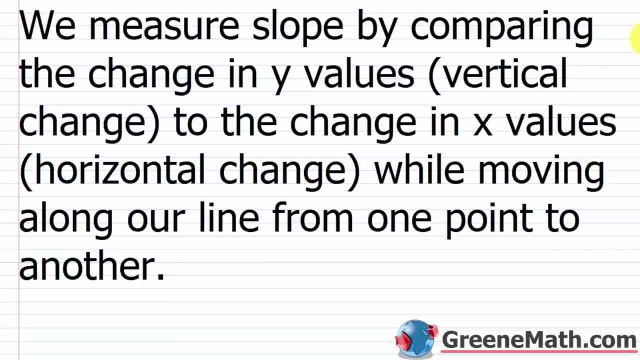 So that's an example of a slope. Alright, so we measure slope by comparing the change in y values, this is the vertical change, remember the y-axis is a vertical axis, to the change in x values, the horizontal change, remember the x-axis is the horizontal axis, while moving along our line from one point to another. 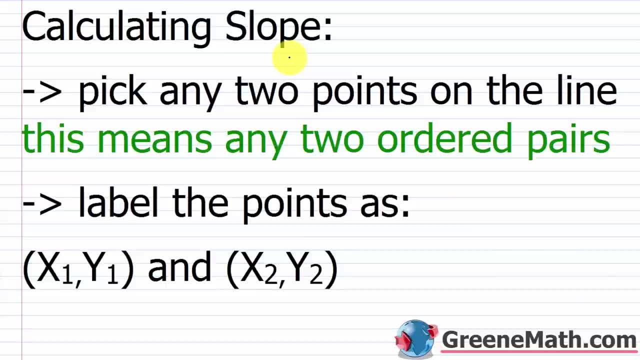 Alright, so how do we actually calculate slope? 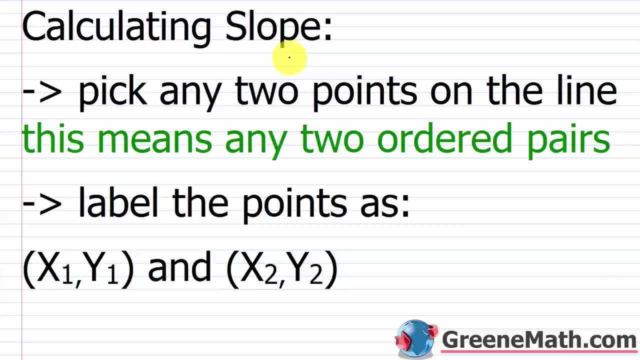 Well, lucky for us, we have something known as the slope formula that we can use. 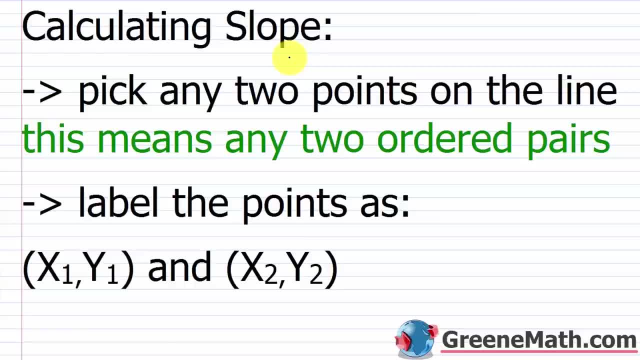 And then we can also do it using the graph which we'll cover in a little while. 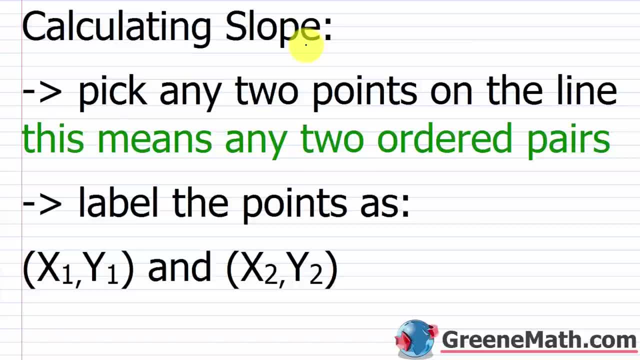 So calculating slope, and this is using the slope formula. You're going to pick any two points on the line. 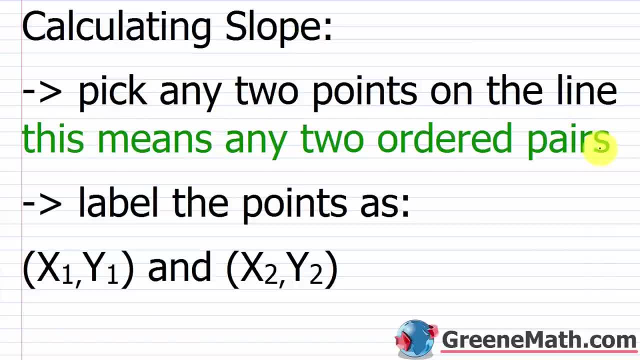 It doesn't matter which two points you pick. So this means any two ordered pairs. And you're going to label the points as x sub 1, y sub 1, 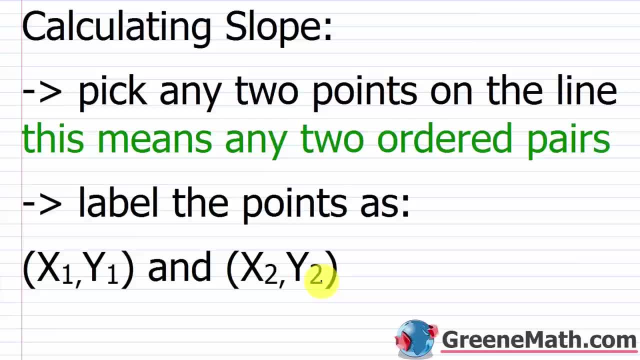 and x sub 2, y sub 2. 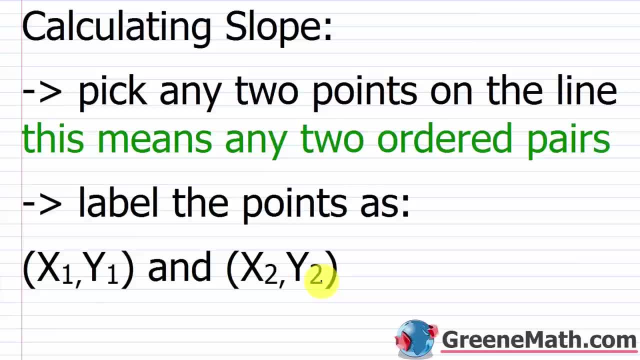 Now let me stop. So I want to clarify. 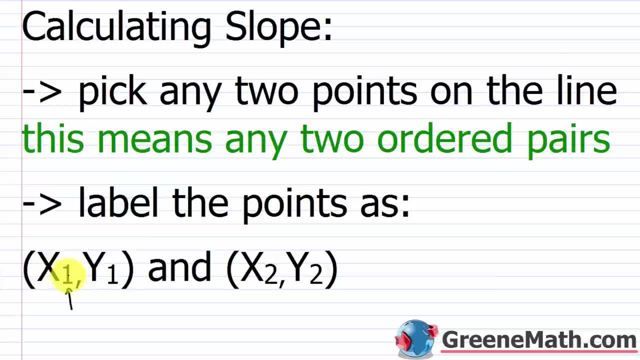 This right here, this one that's kind of sitting next to the x is read as sub 1. 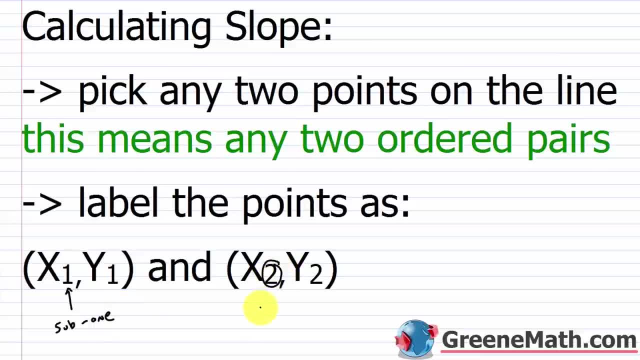 This two that's sitting next to the x is read as sub 2. This is a way for us to notate that we have two different x values 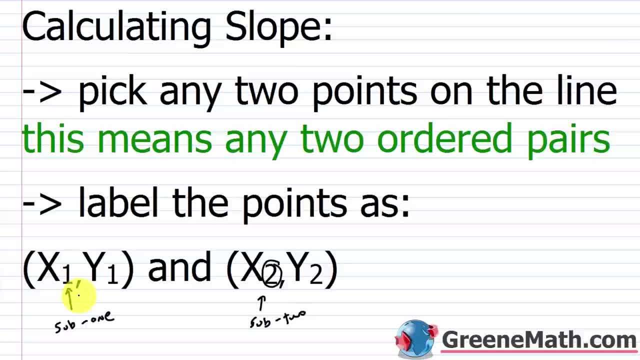 that we're thinking about here without actually kind of changing variables. 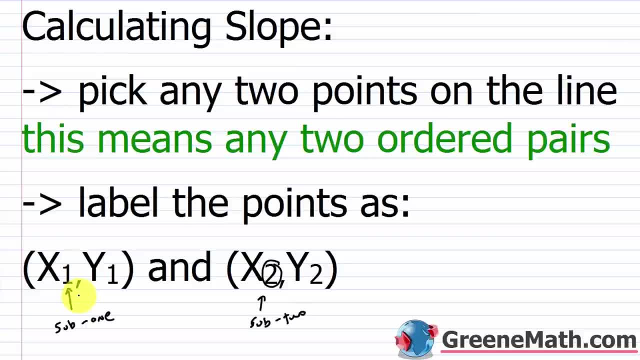 In a lot of math, I can just pick a variable with a different letter every time I have something else I'm representing. 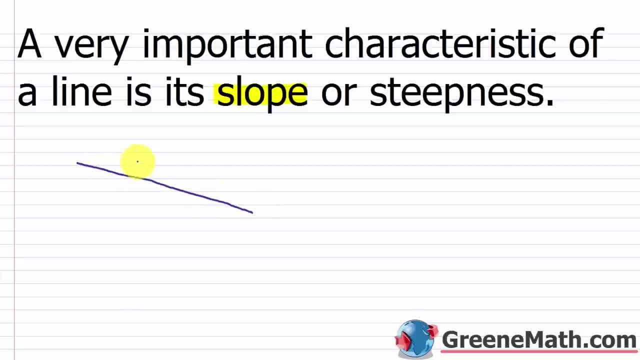 It's slanted downward right. I know that's not a perfectly straight line, but I'm going to draw a picture of a little car here And, just for the record, I am a terrible drawer and I know that. So this is my car here. 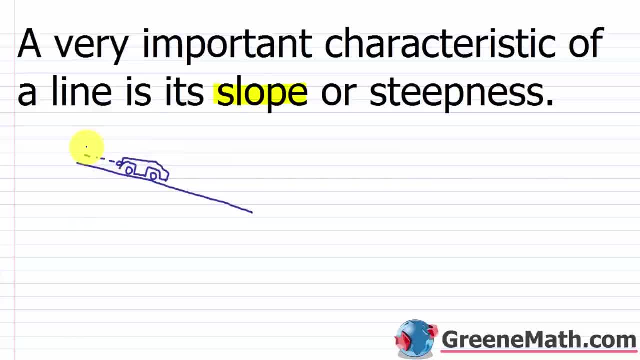 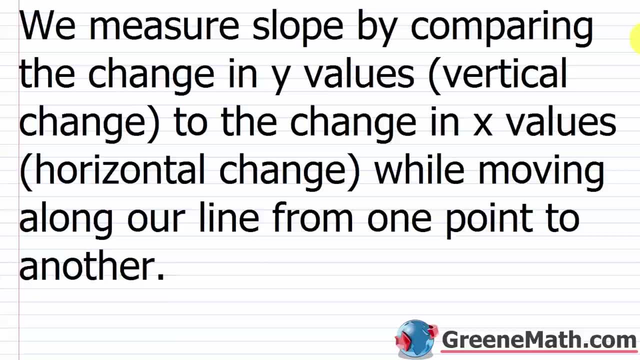 And I'm going to put a little exhaust going out of there And I'm driving and for every 10 miles I go the road is dropping by a mile. So that's an example of a slope. All right, so we measure slope by comparing the change in y values. 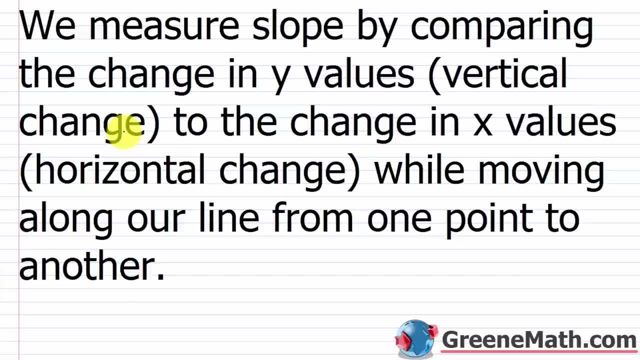 This is the vertical change. Remember the y-axis is a vertical axis to the change in x values. the horizontal change- Remember the x-axis is the horizontal axis while moving along our line from one point to another. All right, so how do we actually calculate slope? 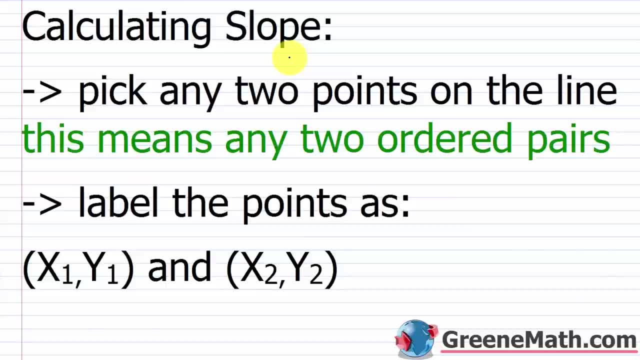 Well, lucky for us, we have something known as the slope formula that we can use, And then we can also do it using the graph, which we'll cover in a little while. So calculating slope, and this is using the slope formula. 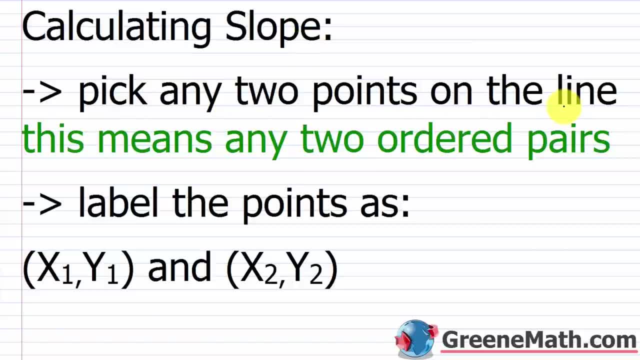 You're going to pick any two points on the line. It doesn't matter which two points you pick. So this means any two ordered pairs, And you're going to label the points as x sub 1, y sub 1, and x sub 2, y sub 2.. 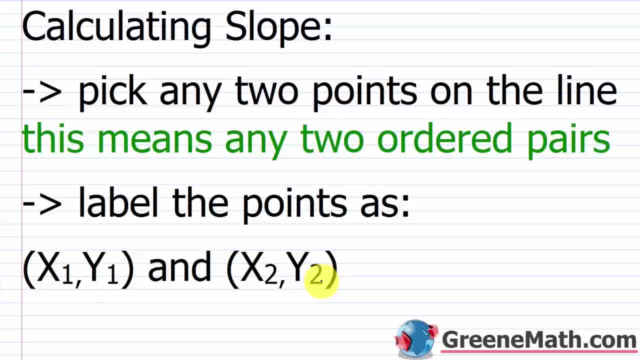 Now let me stop. I'm introducing some new notation, so I want to clarify This right here. this one that's kind of sitting next to the x is read as sub 1.. This 2 that's sitting next to the x. 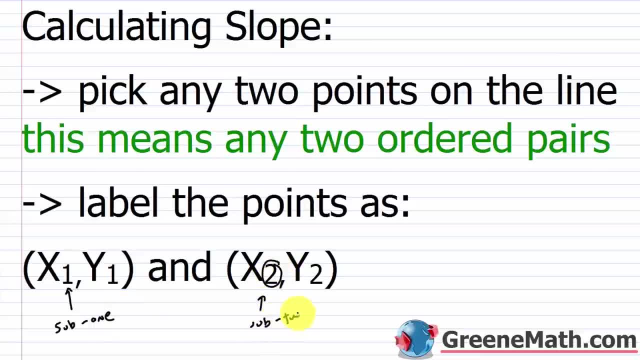 is read as sub 2.. This is a way for us to notate that we have two different x values that we're thinking about here without actually kind of changing variables. right, And in a lot of math I can just pick a variable, a different letter, every time I have something. 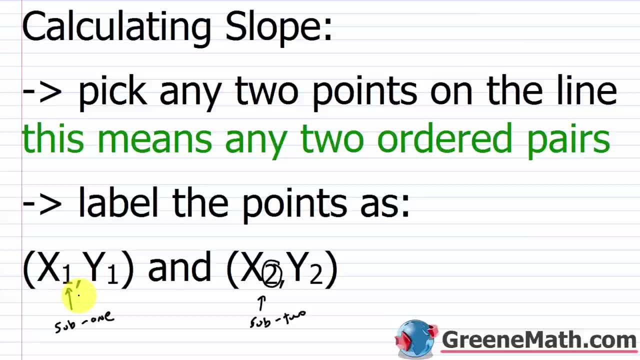 else I'm representing, But here because we're specifically thinking about: OK, the x value is the value that we're thinking about. that corresponds to the horizontal axis. OK, So I've got to be consistent there. I can't say, OK, I have x, and then I have some variable named z. 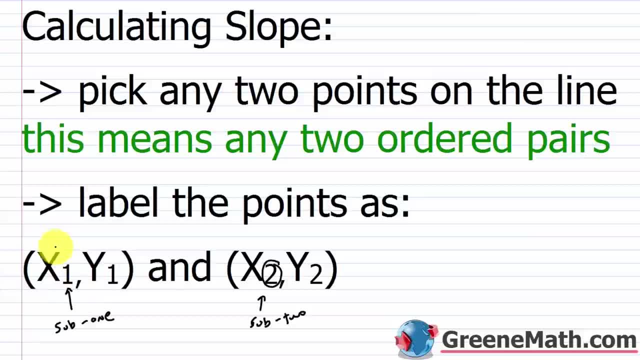 But here, because we're specifically thinking about, okay the x value is the value that we're thinking about that corresponds to the horizontal axis. 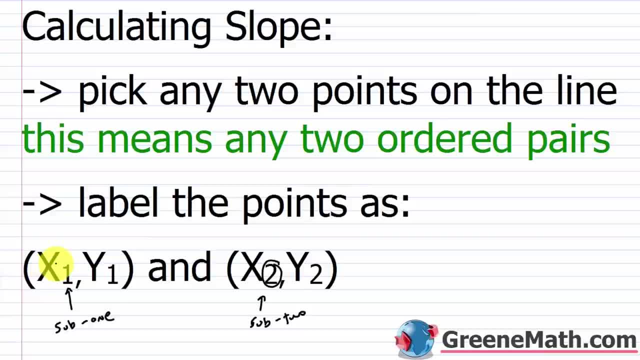 So I've got to be consistent there. I can't say, okay I have x and then I have some variable named z. That wouldn't make any sense. 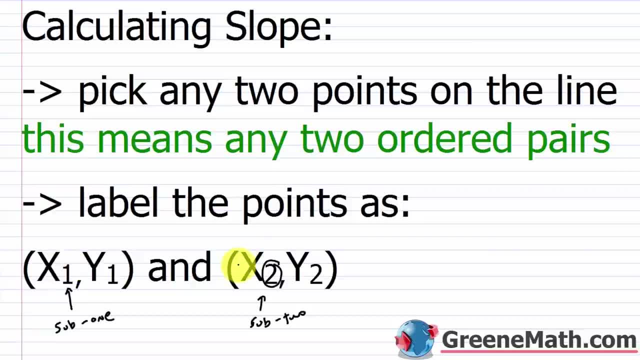 So we have to have two different x values and so to separate them we use sub 1 and sub 2. 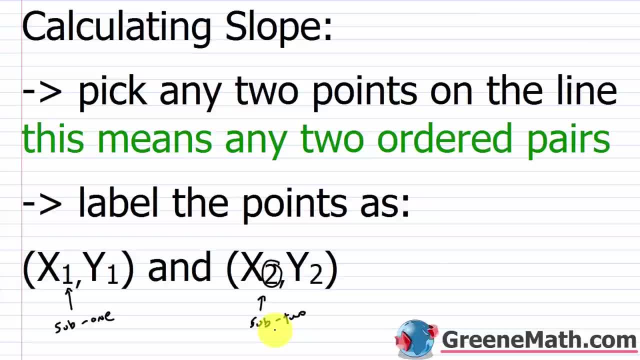 If I was working with something that had three different x values I would have a point that would be x sub 3, y sub 3. 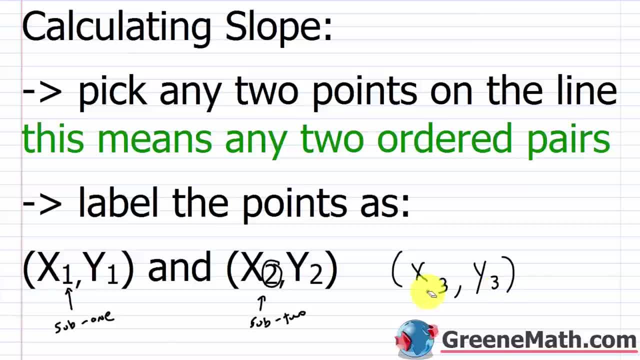 So on and so forth. You're going to see that as you move higher in math when it calls for that. But for right now we just need two. 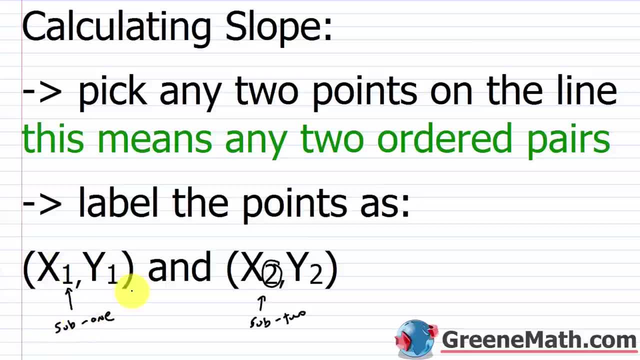 So that's where this is coming from. So you have x sub 1, y sub 1 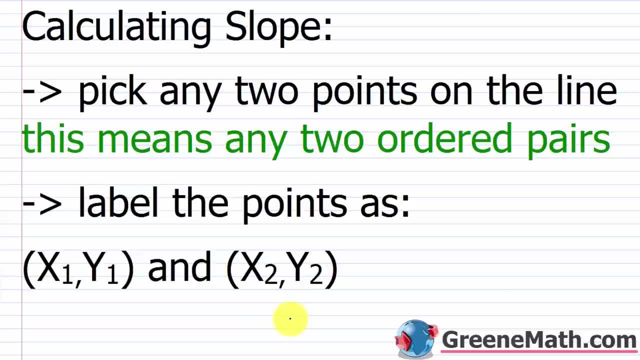 and x sub 2, y sub 2. Now the next source of major confusion 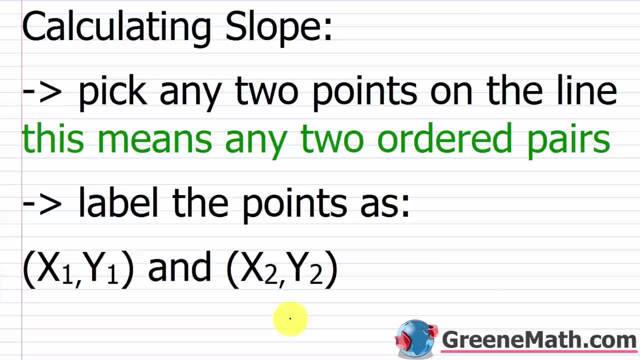 is which point do I label x sub 1, y sub 1 and which point do I label x sub 2, y sub 2. It does not matter. 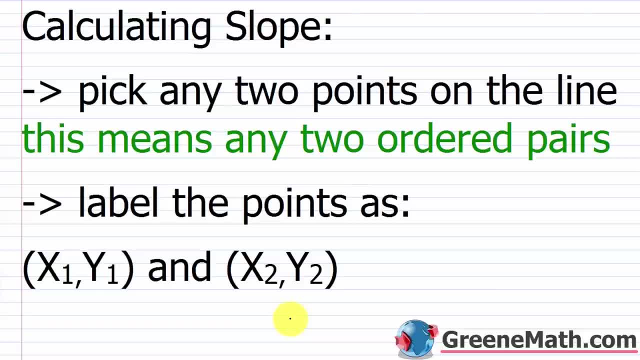 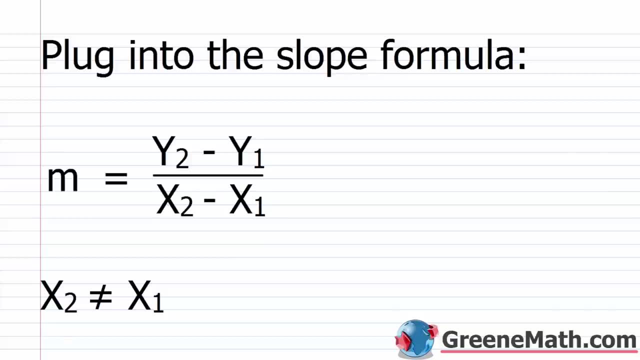 Okay? And I'm going to show you that so that you understand because I can't tell you how many people come up to me and say well how do I know which one to label is which? It does not matter. You can switch them around and you're going to get the same exact answer. So once you've labeled them all you need to do is plug it into the slope formula. 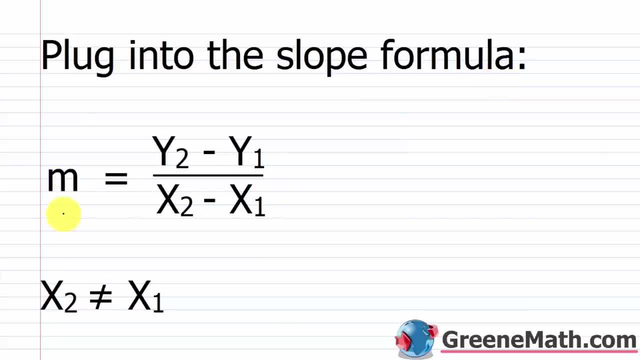 And I advise you to copy this down. We have that m which stands for 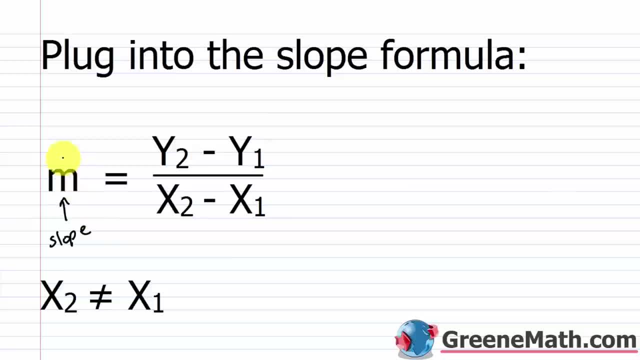 slope. This stands for slope. m stands for slope but it does. 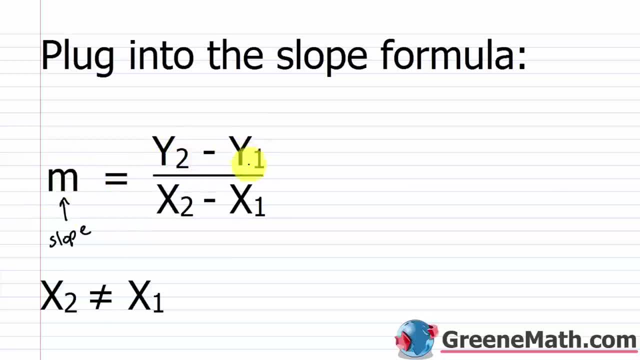 And this is equal to we have y sub 2 minus y sub 1. 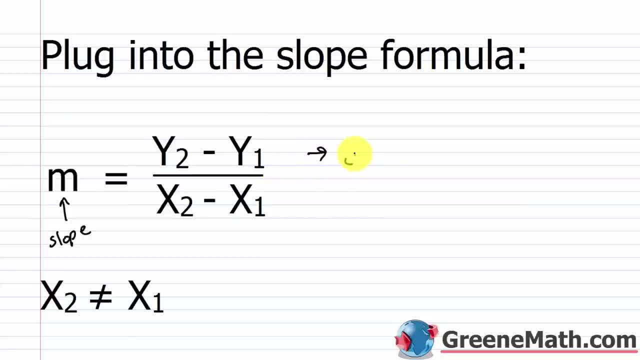 So this is referred to as your change your change in y values. 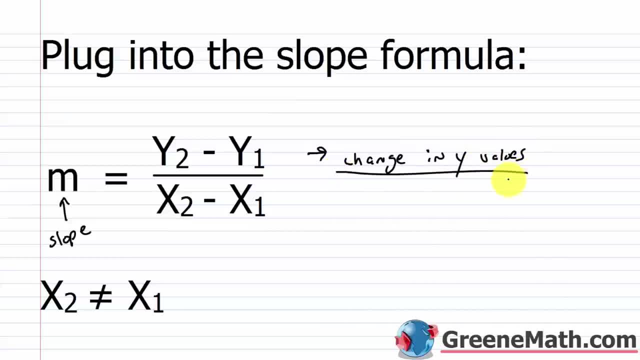 And then this is over or you can think about it as dividing by x sub 2 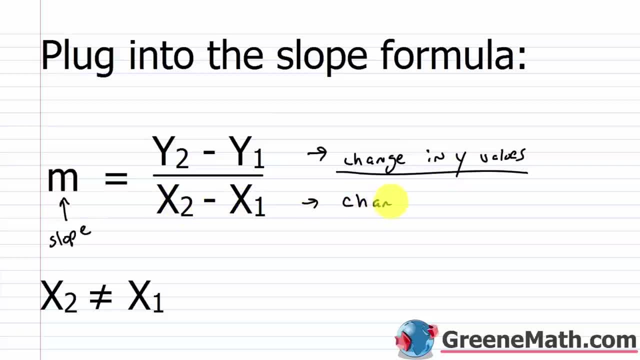 minus x sub 1 which is what? It's the change in x values. 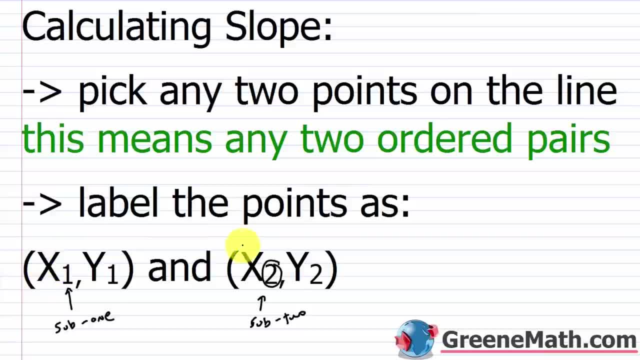 That wouldn't make any sense. So we have to have two different x values, And so to separate them we use sub 1 and sub 2.. If I was working with something that had three different x values, I would have a point that 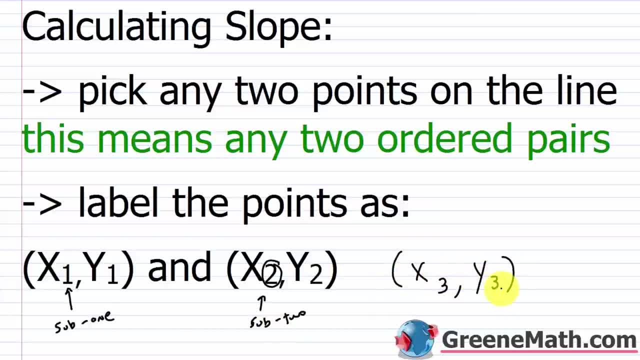 would be x sub 3, y sub 3, right, So on and so forth, And you're going to see that as you move higher in math when it calls for that. But for right now we just need x. OK. 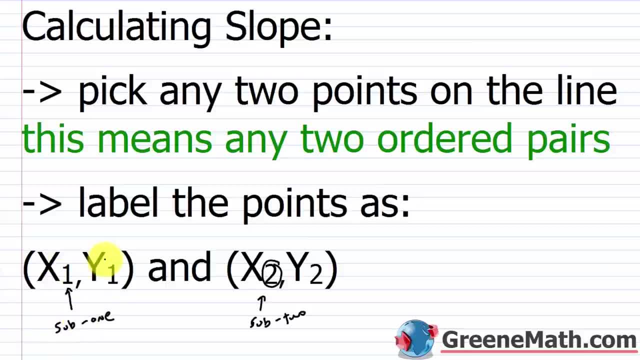 We just need 2.. So that's where this is coming from. So you have x sub 1, y sub 1, and x sub 2, y sub 2.. Now the next source of major confusion is: which point do I label x sub 1, y sub 1?? 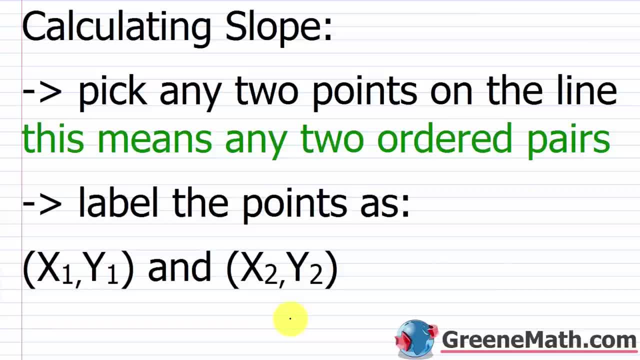 And which point do I label x sub 2, y sub 2?? And the answer is: it does not matter. OK, And I'm going to show you that so that you understand, Because I can't tell you how many people come up to me and say: well, how do I know which? 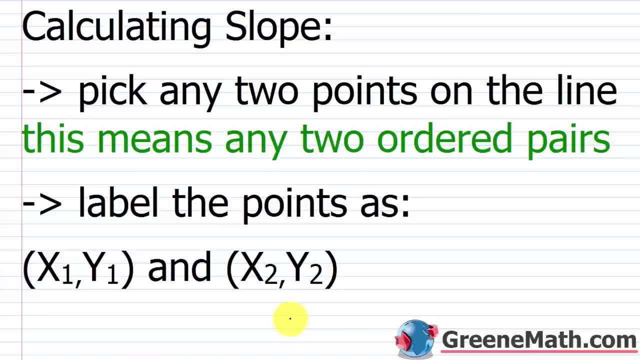 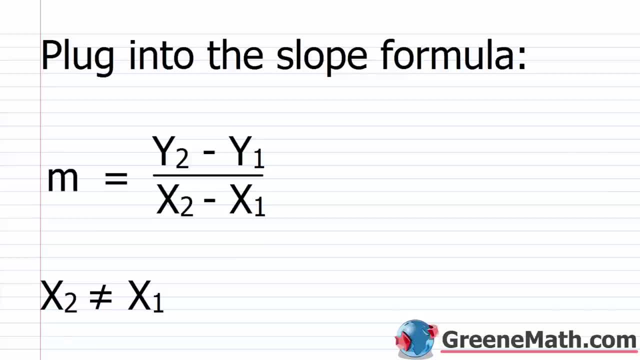 one to label, as which It does not matter. You can switch them around. You're going to get the same exact answer. So once you've labeled them, all you need to do is plug it into the slope formula, And I advise you to copy this down. 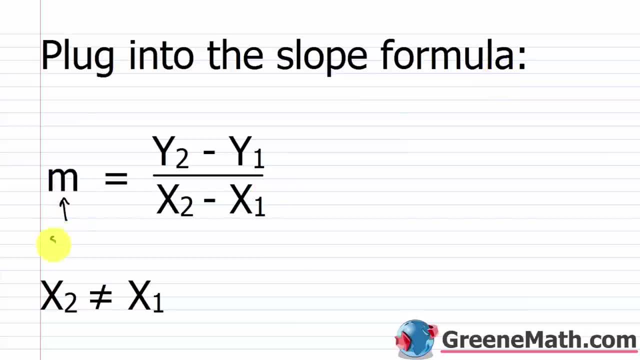 We have that m which stands for slope. This stands for slope, And I don't know why m stands for slope, but it does. And this is equal to: we have y sub 2 minus y sub 1.. So this is referred to as your change. 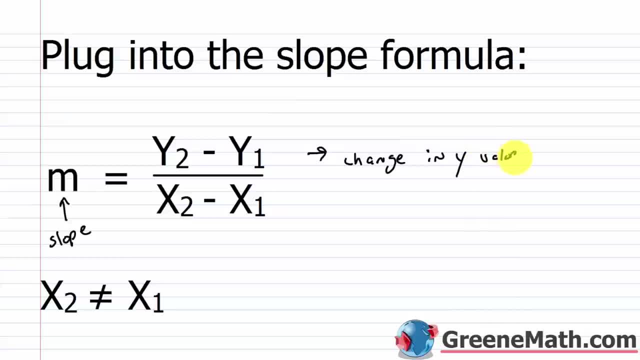 Your change in y Y values, And then this is over. we can think about it as dividing by x sub 2 minus x sub 1, which is what It's: the change in x values, The change in x values. 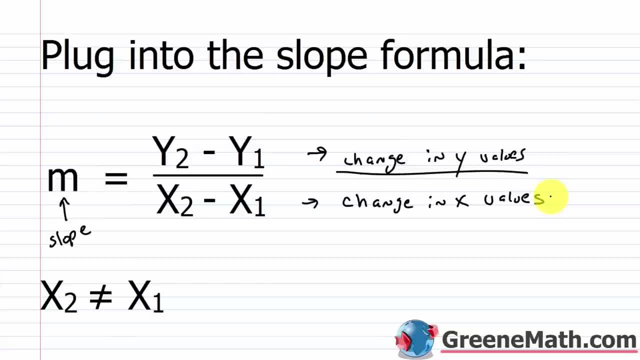 So we have the change in y values over the change in x values. And then one important note: we can never have the case where x sub 2 equals x sub 1.. Why? Because we can't divide by 0. If I have the same number here, let's say 2 and 2, 2 minus 2 is 0, I can't divide by. 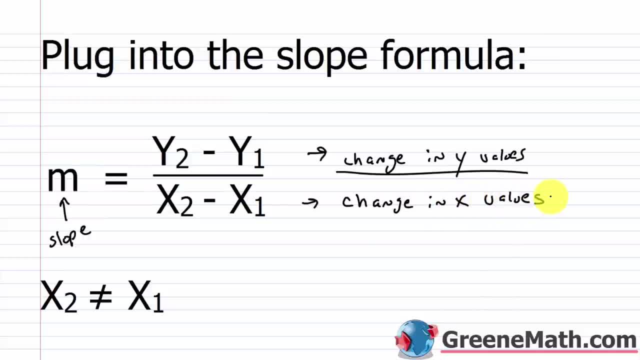 Okay? The change in x values. 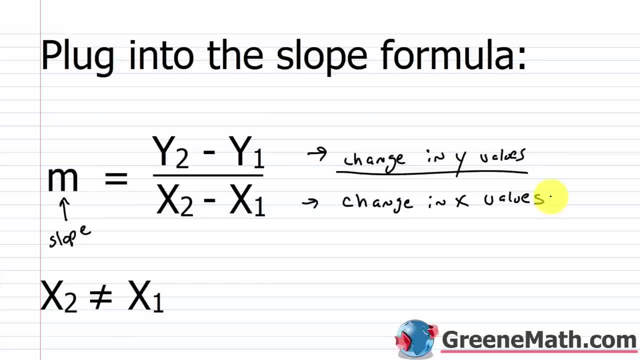 So we have the change in y values over the change in x values. 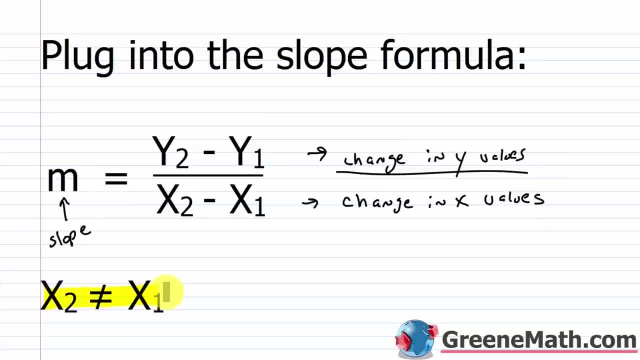 And then one important note, we can never have the case where x sub 2 equals x sub 1. Why? Because we can't divide by 0. 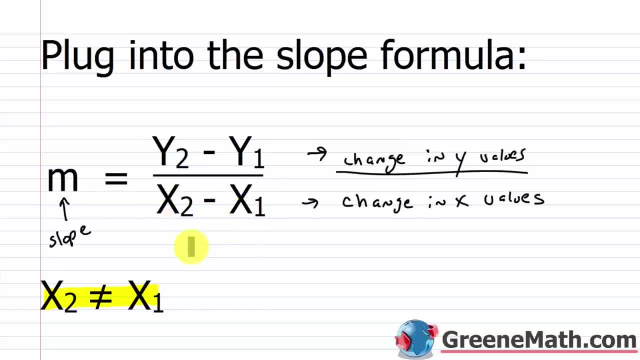 If I have the same number here, let's say 2 and 2, 2 minus 2 is 0 I can't divide by 0. So that's a problem. 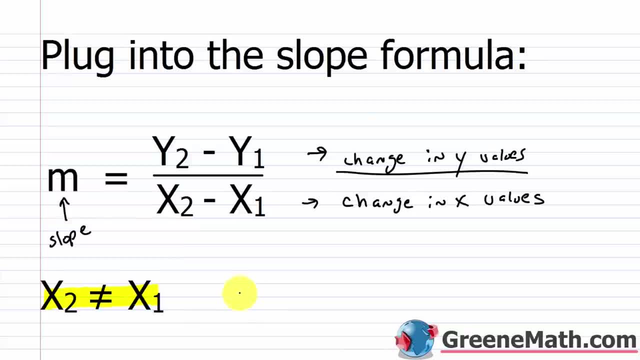 So x sub 2 cannot equal x sub 1. And another way we might see this written is that m, our slope 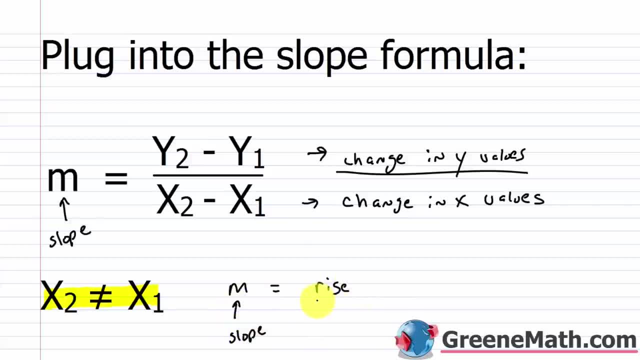 is equal to the rise over the run. 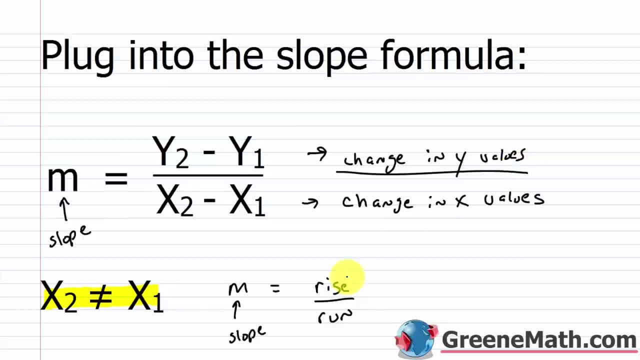 And this is just a way to remember that it's the change in y values or the rise, you can kind of think about this as going up and down, over the change in x values or the run. 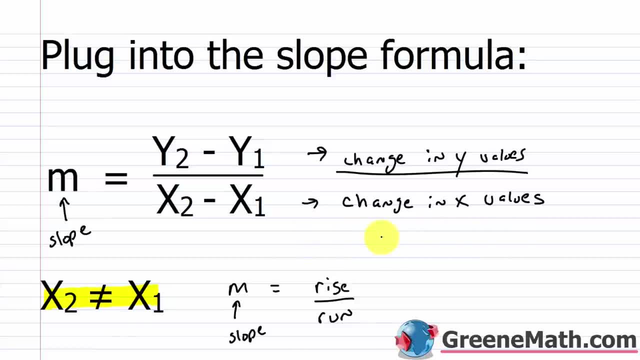 You can kind of think about running as going sideways or horizontally being on that horizontal x axis. Alright, so let's start out 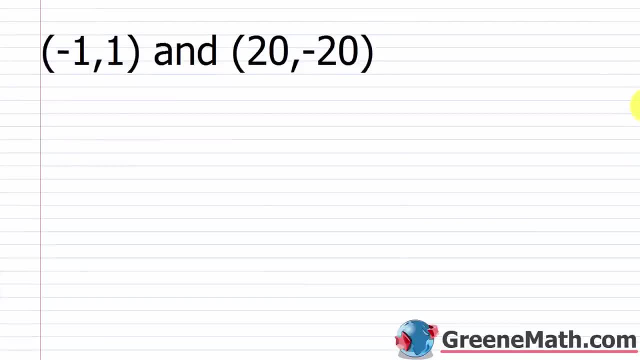 with two points. This is a typical example of something you see on your homework or test. You're given two points and you're asked to calculate the slope. 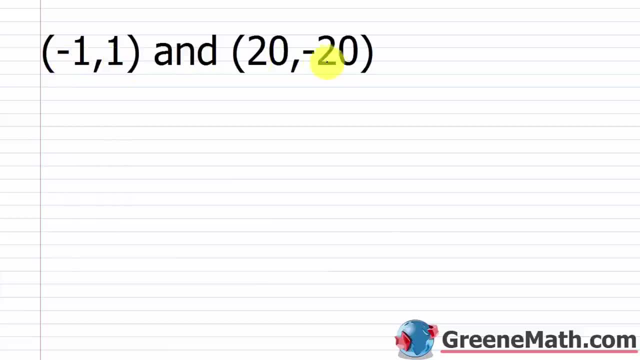 So we have the point and . 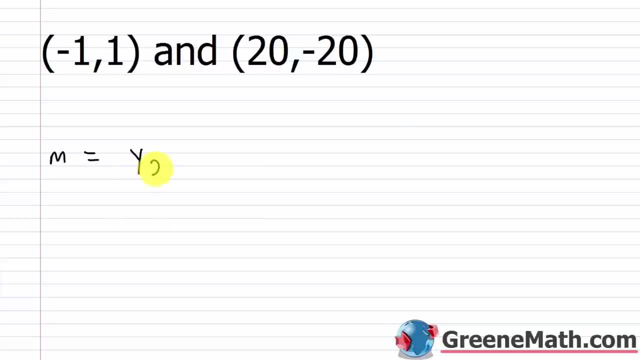 So the slope formula is m equals y sub 2 minus y sub 1 over x sub 2 minus x sub 1 and I'm not going to write this every time but remember that x sub 2 is not allowed to equal x sub 1. It cannot. All we need to do is label one of these points as x sub 1, y sub 1 and the other x sub 2, y sub 2 and then just plug in. 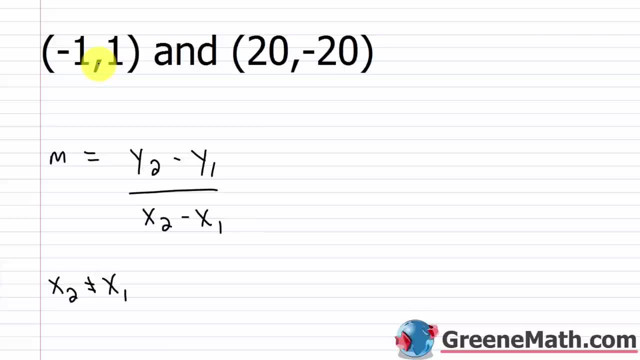 Again, it does not matter. Which point you choose to be x sub 1, y sub 1 and which point you choose to be x sub 2, y sub 2. It's completely irrelevant. You get the same answer either way. So I'm going to pick this to be x sub 1, y sub 1 and I'm going to pick this to be x sub 2, y sub 2. 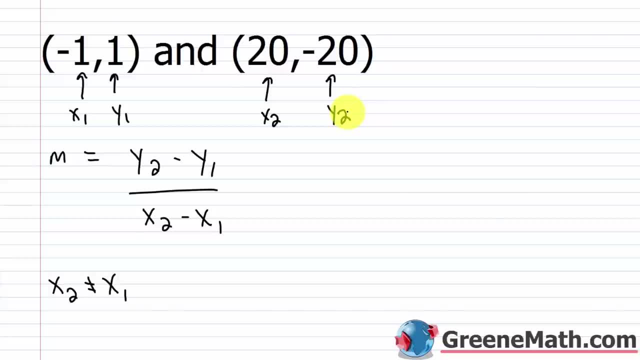 One thing that you cannot do you cannot mess this up in terms of saying this is x sub 1, y sub 2 and this is x sub 2, y sub 1. 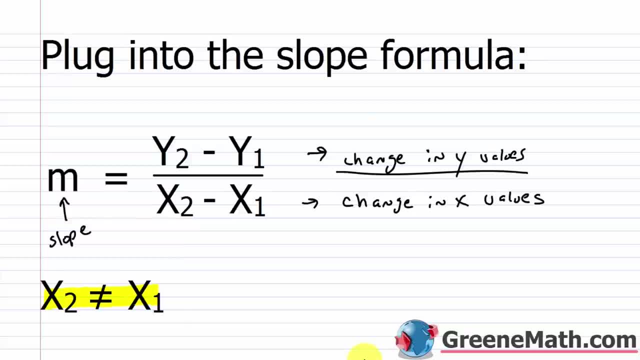 0.. So that's a problem. So x sub 2 cannot equal x sub 1.. And another way we might see this written is that m, our slope, is equal to the rise over the run, And this is just a way to remember that it's the change in y values, or the rise, you can. 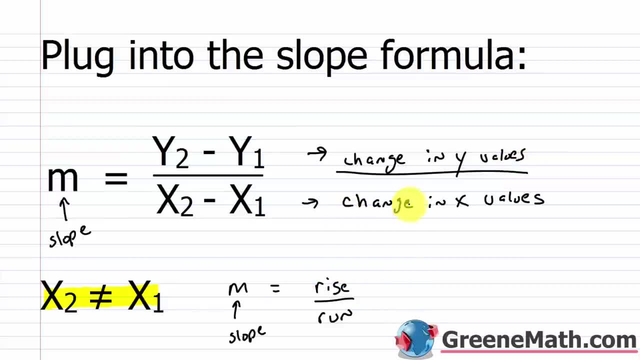 kind of think about this as going up and down, Or the change in x values or the run. You can kind of think about running as going sideways Or horizontally, being on that horizontal x axis. All right, so let's start out with two points. 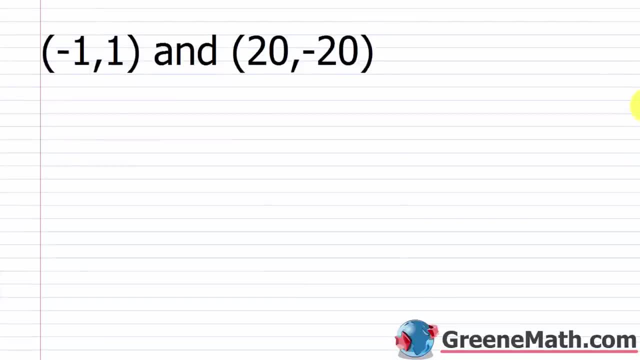 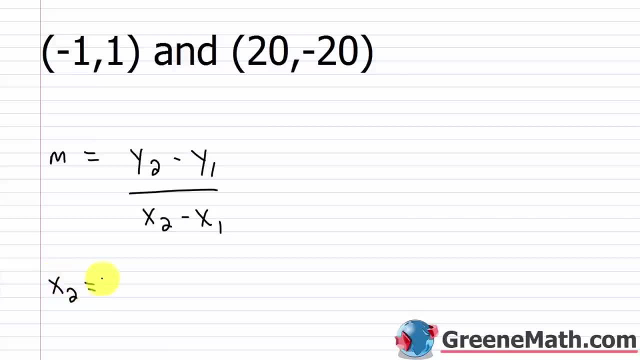 Over. I'm not going to write this every time, but remember that x sub 2 is not allowed to equal x sub 1.. It cannot. All we need to do is label one of these points as x sub 1,, y sub 1, and the other x sub 2,. 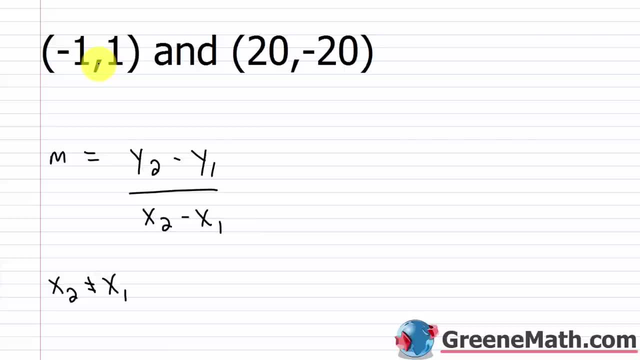 y sub 2, and then just plug in Again. it does not matter which point you choose to be x sub 1, y sub 1, and which point you choose to be x sub 2, y sub 2.. It's completely irrelevant. 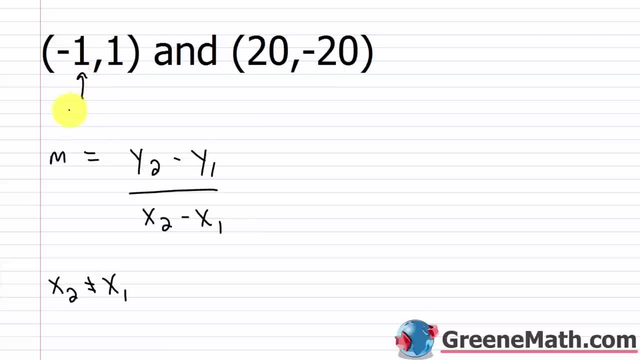 You get the same answer either way. I'm going to pick this to be x sub 1, y sub 1, and I'm going to pick this to be x sub 2, y sub 2.. One thing that you cannot do: you cannot mess this up in terms of saying, well, this is. 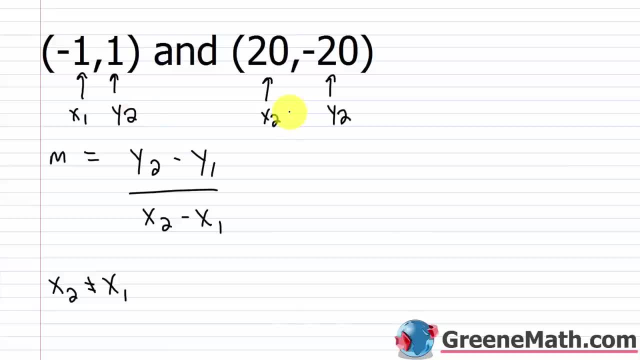 x sub 1, y sub 2, and this is x sub 2, y sub 1.. That will give you the wrong answer. Do not do that. If this is x sub 1,, this has to be y sub 1.. 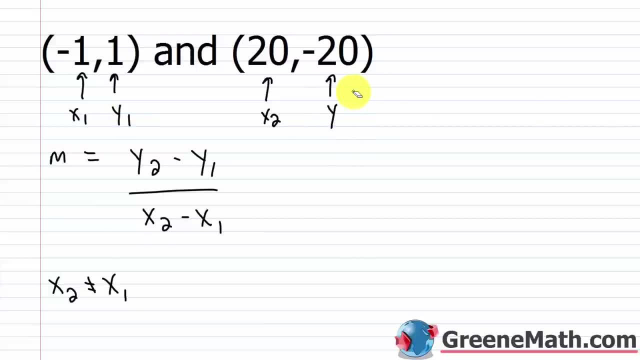 If this is x sub 2, this has to be y sub 2.. You cannot mix those numbers up like that. Once you have labeled everything, go ahead and just plug into the slope formula. It's really just that simple. I have y sub 2 here, so I'm going to take negative 20 and plug that in. 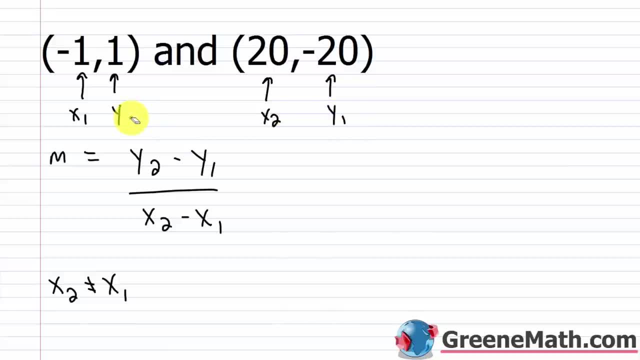 I'm going to give you the wrong answer. Do not do that. If this is x sub 1, this has to be y sub 1. 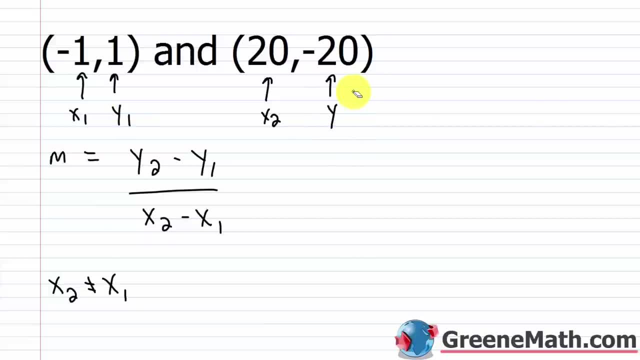 If this is x sub 2, this has to be y sub 2. 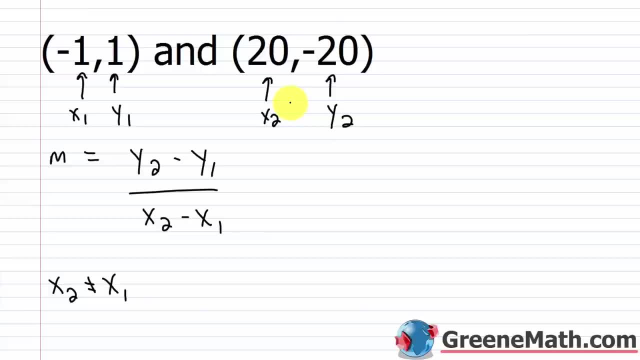 You cannot mix those numbers up like that. 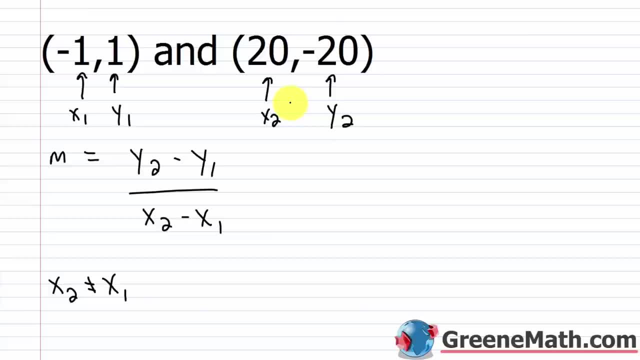 Now once you have labeled everything go ahead and just plug into the slope formula. It's really just that simple. 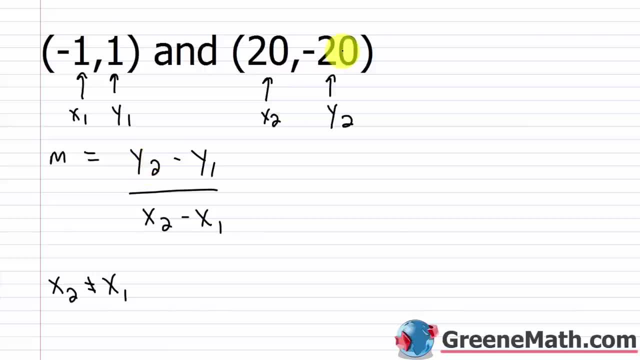 So I have y sub 2 here. So I'm going to take negative 20 and plug that in. So let me just erase this and just put a negative 20 here in its place. 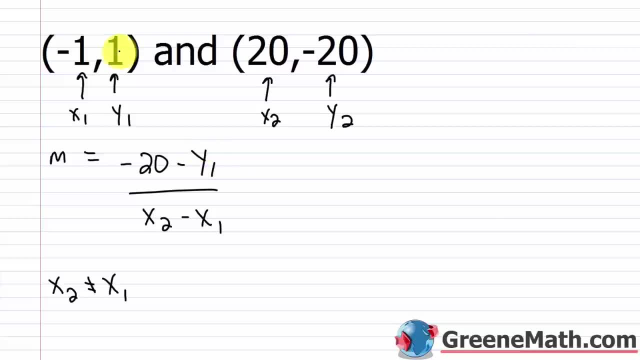 And then I have minus. I have y sub 1. So that's 1. Let's erase this and put 1. And then I have x sub 2 down here. That's 20. So erase this and put 20. And then for x sub 1 I have negative 1. So let's erase this and put a negative 1. Now again, again, again. 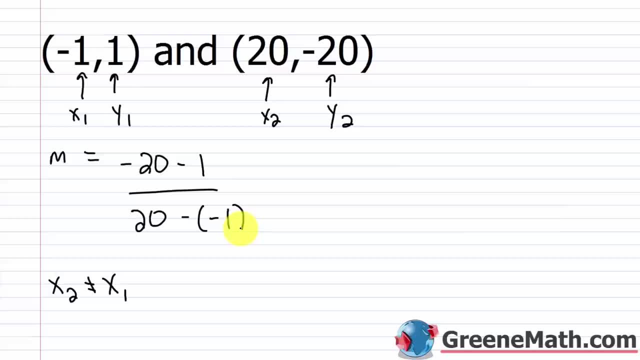 It's very important to pay attention to your signs when you're plugging in for something. I already had a negative out in front. I'm plugging in a negative 1 for x sub 1. So it's minus a negative 1. Don't make the silly mistake of just seeing that out in front and just putting minus 1. You get the wrong answer. So then all I need to do now is just simplify. I have negative 20 minus 1 which is negative 21. 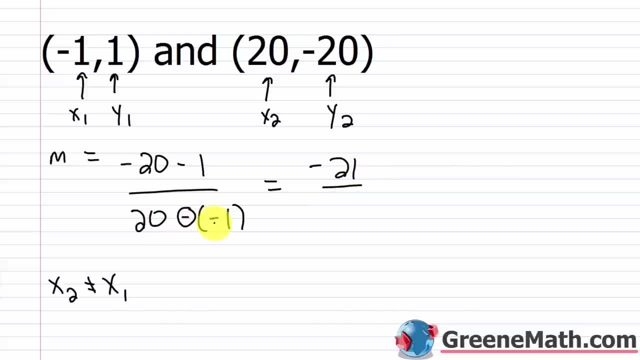 And this is over 20 minus a negative 1 which is the same thing as 20 plus 1 which is 21. 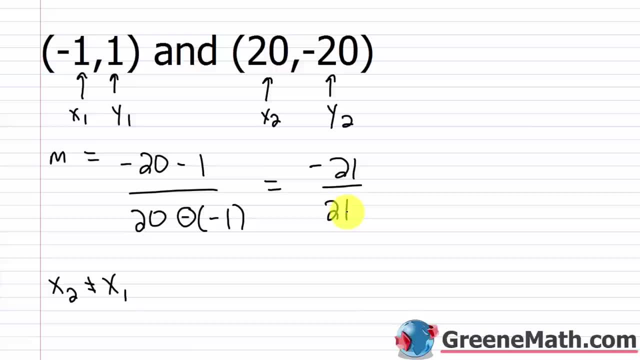 So I end up with negative 21 over 21 which is the same thing as negative 1. 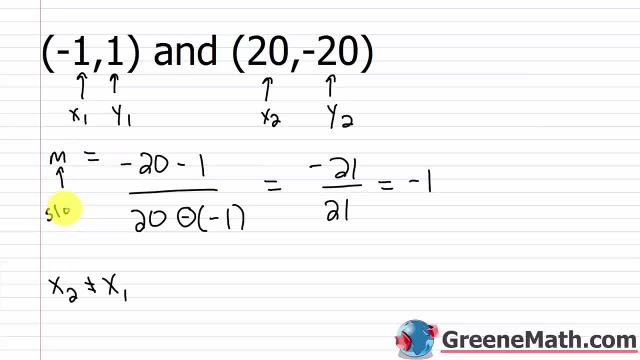 So m, again my slope, let me label that real quick, my slope is equal to negative 1. 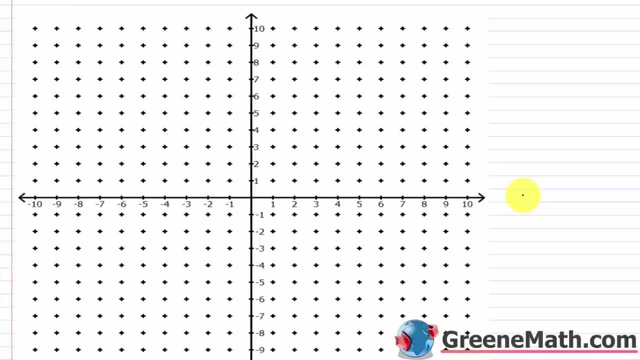 So let's see if we can make a little sense out of this slope thing. 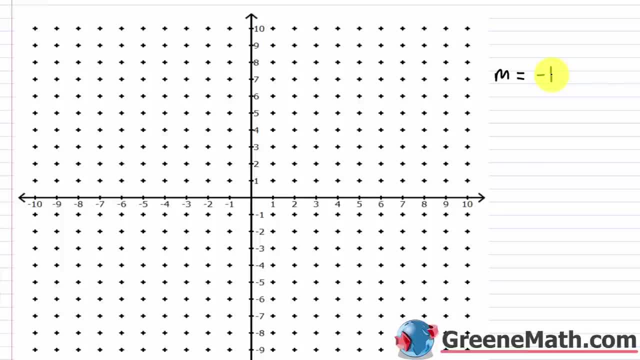 So we saw that m is equal to negative 1. So what does that mean? 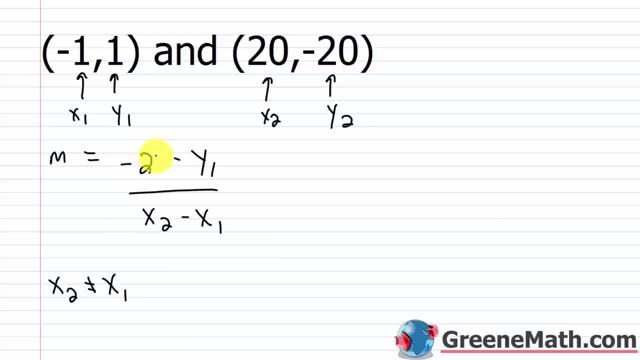 Let me just erase this and just put a negative 20 here in its place. Then I have minus. I have y sub 1.. That's 1.. Let's erase this and put 1.. Then I have x sub 2 down here. 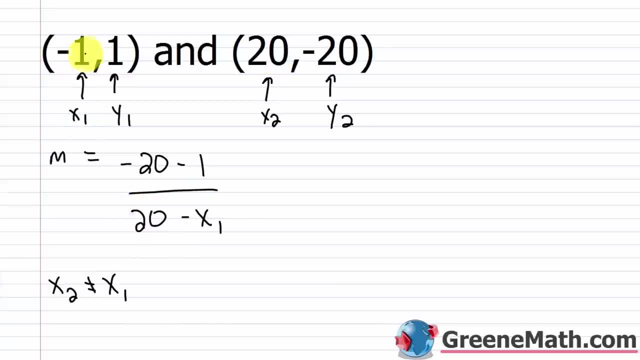 That's 20.. Erase this and put 20.. Then for x sub 1, I have negative 1.. Let's erase this and put a negative 1.. Again, again, again. it's very important to pay attention to your signs when you're plugging. 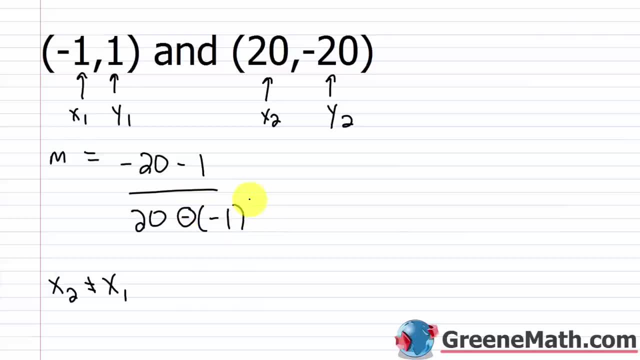 in for something. I already had a negative out in front. I'm plugging in a negative 1 for x sub 1, so it's minus a negative 1.. Don't make the silly mistake of just seeing that out in front and just putting minus 1.. 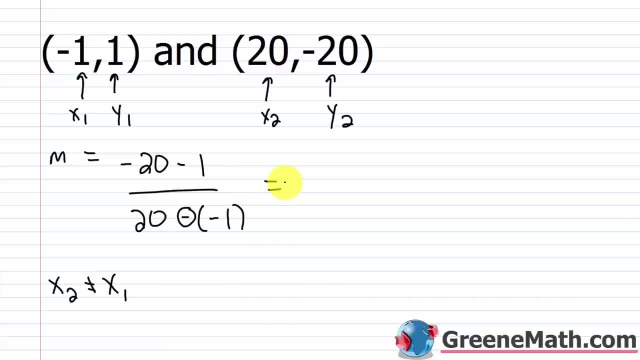 You get the wrong answer, Then all I need to do now is just simplify. I have negative 20 minus 1,, which is negative 21.. This is over 20 minus a negative 1,, which is the same thing as 20 plus 1,, which is 21.. 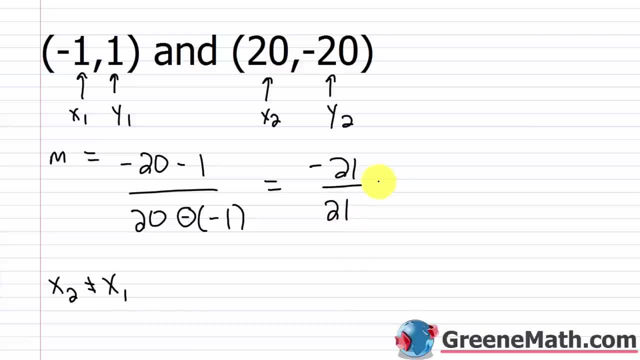 I end up with negative 21 over 21,, which is the same thing as negative 1.. M again, my slope. let me label that real quick. my slope is equal to negative 1.. Let's see if we can make a little sense out of this slope thing. 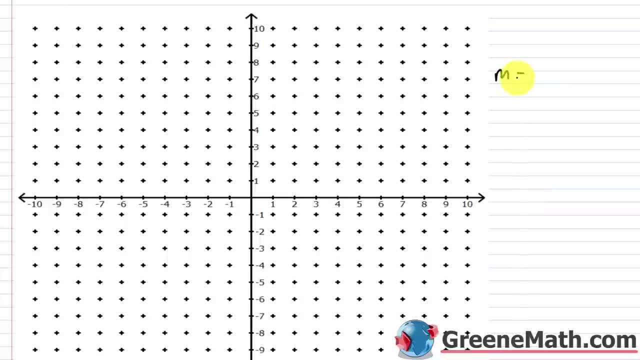 We saw that M is equal to negative 1.. What does that mean? Again, if you look at the rise over run explanation- so rise over run- we know that we can write negative 1 as negative 1 over 1.. That's the same thing. 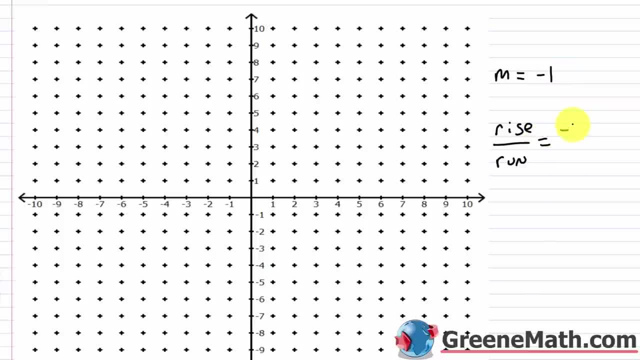 If you divide by 1, it's just itself. I can put this as equal to negative 1 over 1.. I look at what's in the numerator. I have rise here. I have negative 1.. I have negative 1 here. 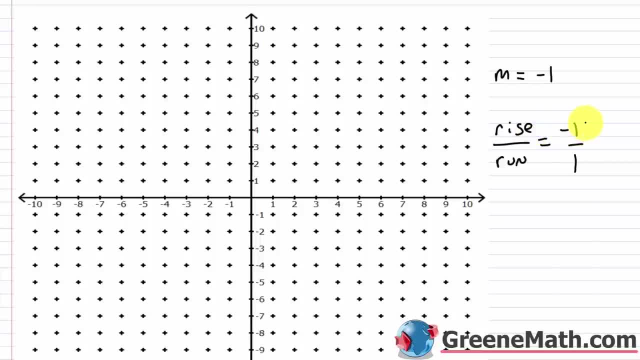 That means I'm going to rise by negative 1 or fall by 1 unit for every run, which we think of as going sideways by 1 unit, Because this is positive down in the run. that means I'm going to the right. 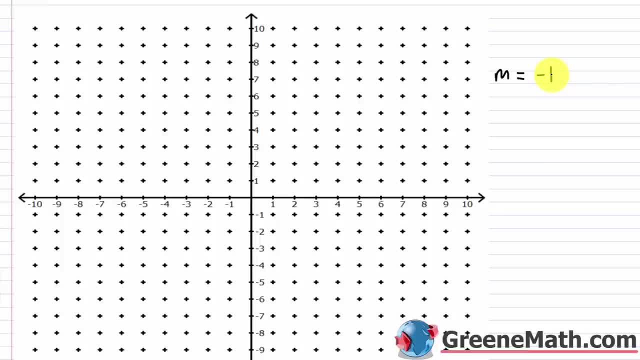 Well again if you kind of look at the rise over run explanation. So rise over run. We know that we can write negative 1 as negative 1 over 1. Right? That's the same thing. If you divide by 1 it's just itself. 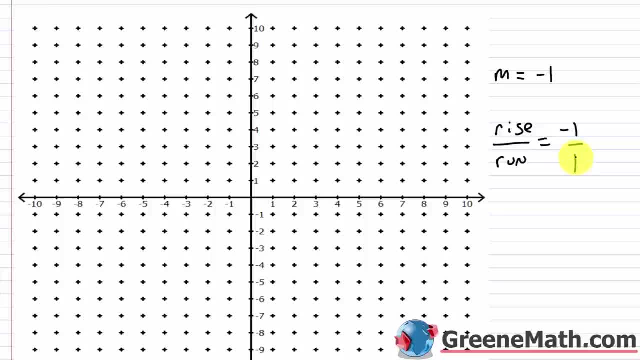 So I can put this as equal to negative 1 over 1. So I look at what's in the numerator. I have rise here and I have negative 1 here. So that means I'm going to rise by negative 1 or fall by 1 unit for every run which we think of as going sideways by 1 unit. 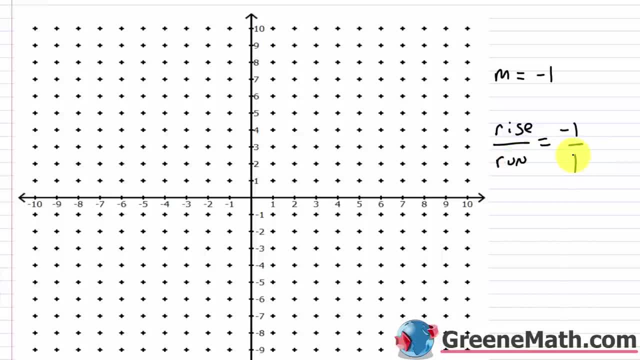 Now because this is positive down in the run that means I'm going to the right. So positive in terms of the x axis means you go right. Negative means you go left. Positive in terms of the y axis means you go up. Negative means you go down. So if I started out at a point on this line. So we know that 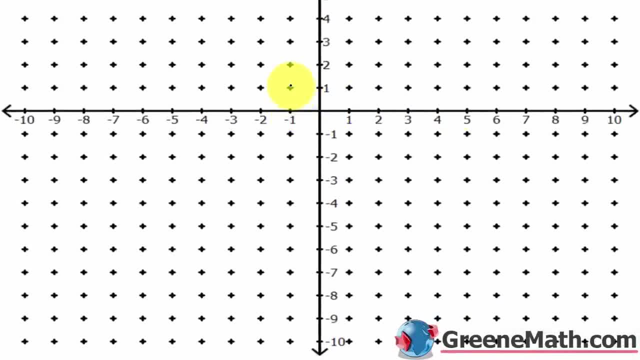 negative 1 comma 1 which is going to be right here. 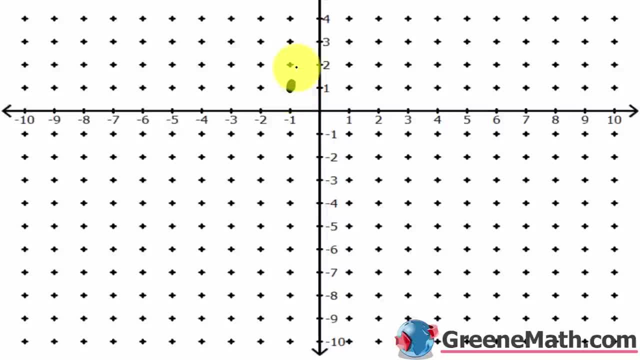 So that's a point on the line. I could actually use this to graph the line. Because I know that I'm going to fall by 1 unit. So I'm going to fall by 1 unit thinking about the rise for every 1 unit I go to the right. So I'm going to go down 1 and over to the right 1. So this point would be on that line. And I can keep doing that. I can go down 1 to the right 1. And go down 1 to the right 1. 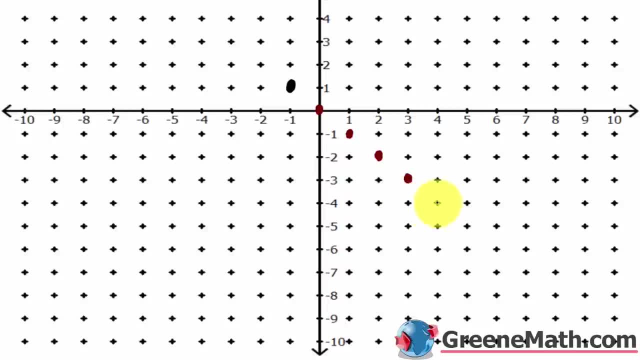 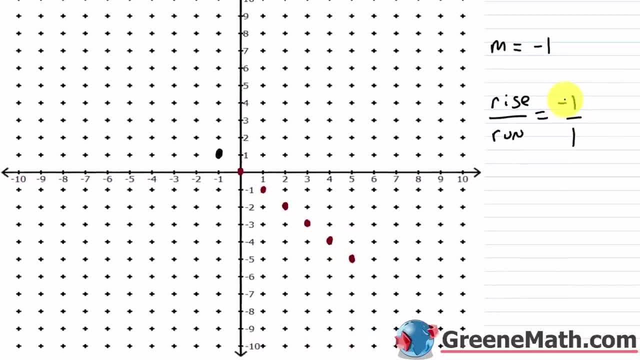 thing I can do. Remember when we're dividing and we think about having a negative in the numerator but a positive in the denominator I can legally switch that. 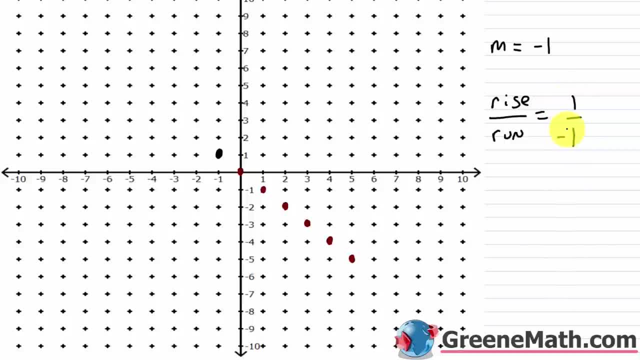 And I can legally say that this is 1 divided by negative 1. Now how would we read that? 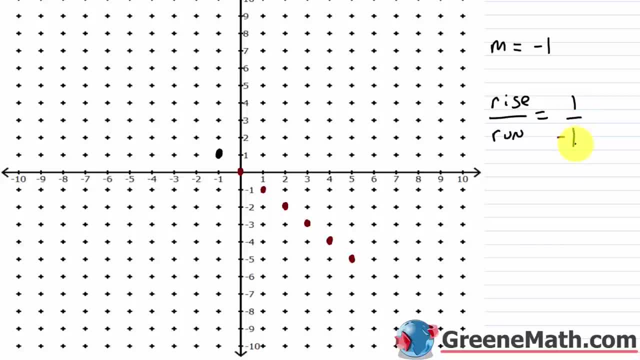 Well that means that we would rise 1 unit for every 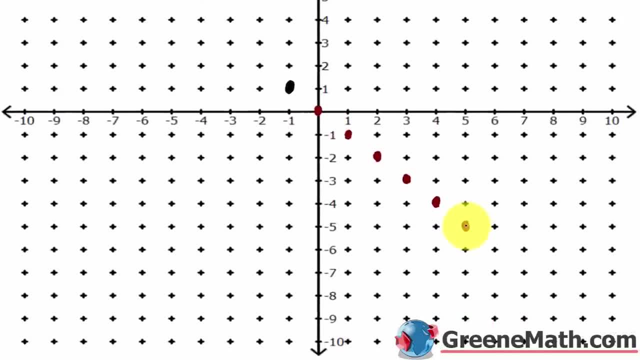 unit we go to the left on the x axis. So starting out at this point 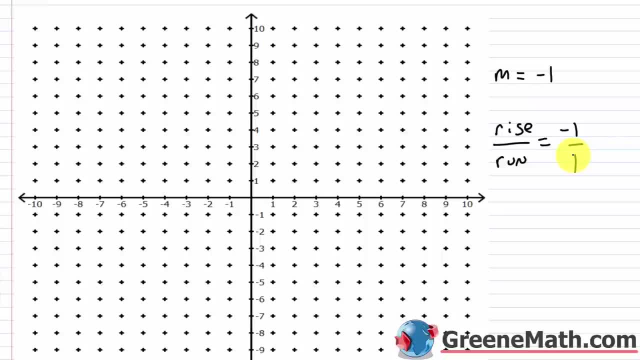 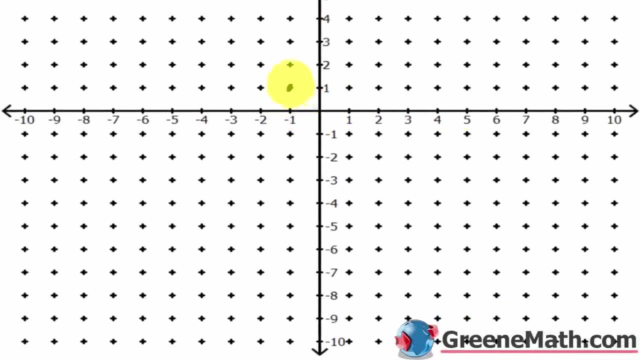 Positive in terms of the x-axis means you go right. Negative means you go left. Positives in terms of the y-axis means you go up. Negative means you go down. If I started out On this line, So we know that negative 1 comma 1, which is going to be right here. 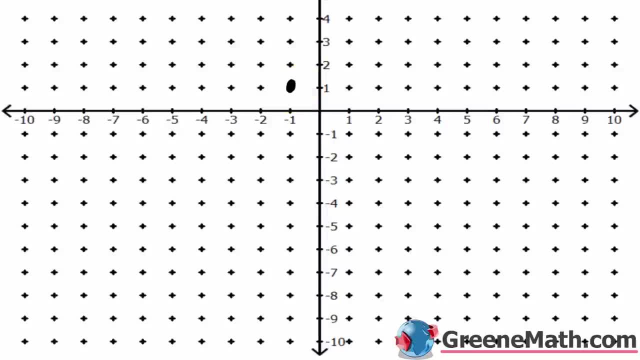 So that's a point on the line. I could actually use this to graph the line, Because I know that I'm going to fall by 1 unit. So I'm going to fall by 1 unit. thinking about the rise for every 1 unit, I go to the right. 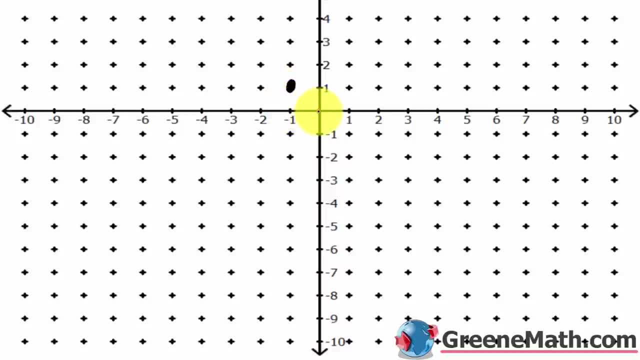 So I'm going to go down 1 and over to the right 1.. So this point would be on that line. I can keep doing that. I can go down 1 to the right And go down 1 to the right 1.. 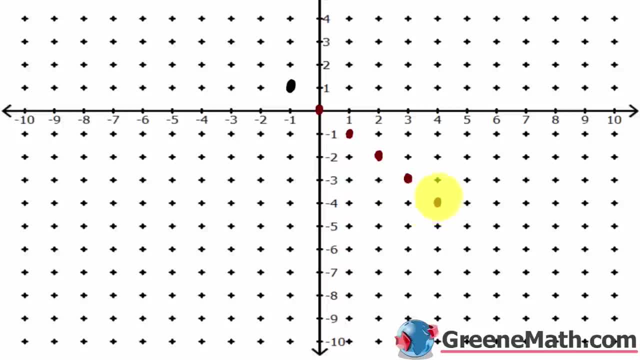 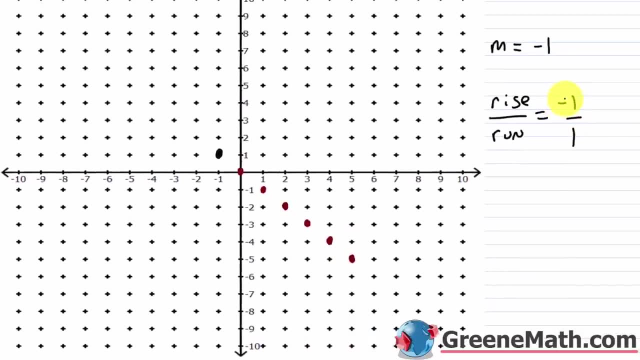 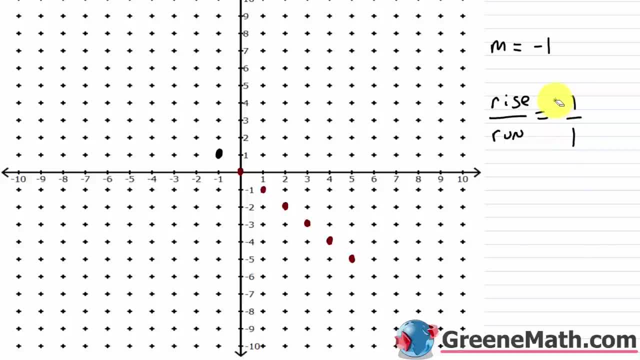 I can legally switch that. I can legally say that this is 1 divided by negative 1.. Now how would we read that? Well, What I can do is that we would rise 1 unit for every unit we go to the left on the x-axis. 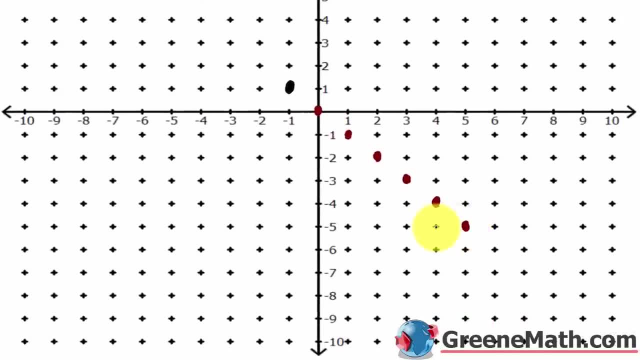 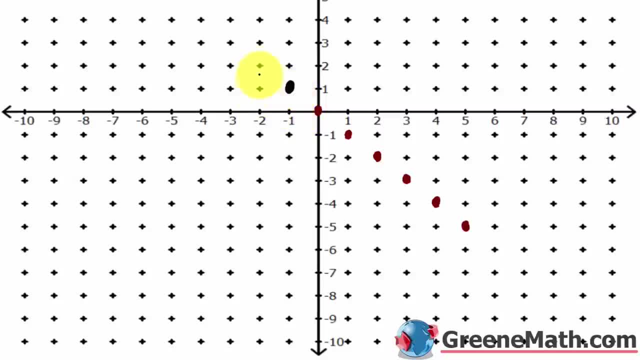 Left 1 up, 1.. Left 1 up, 1.. I can keep going: Left 1 up, 1.. Here's another point: Left 1 up, 1.. Here's another point, And you can see that I can easily draw a completely straight line through those points. 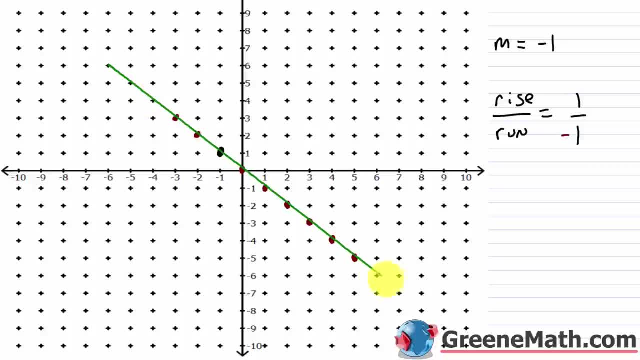 And let me do that real quick- Not perfectly straight, but you get the idea, And later on we're going to learn how to take this information that we have and find the equation for the line. So this is actually: y equals negative x, And I know that you don't know how to do that yet. 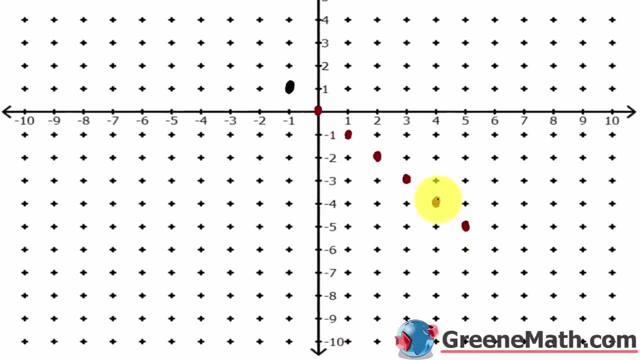 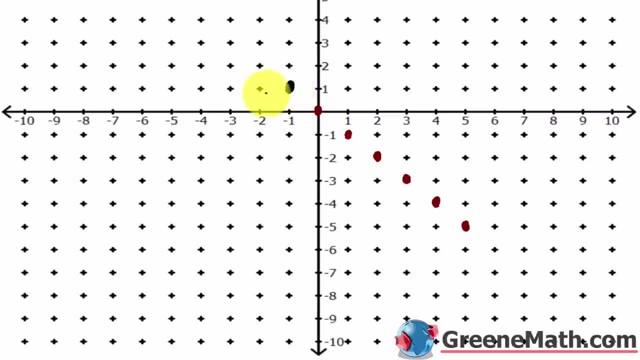 Left 1 up 1. Left 1 up 1. I can keep going. Left 1 up 1. Here's another point. Left 1 up 1. Here's another point. You can see that I can easily draw a completely straight line through those points. And let me do that real quick. Not perfectly straight but you get the idea. 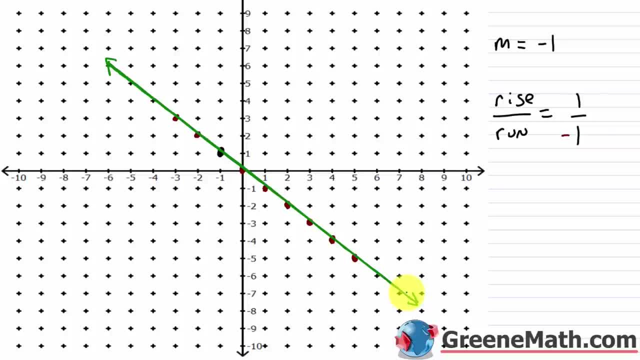 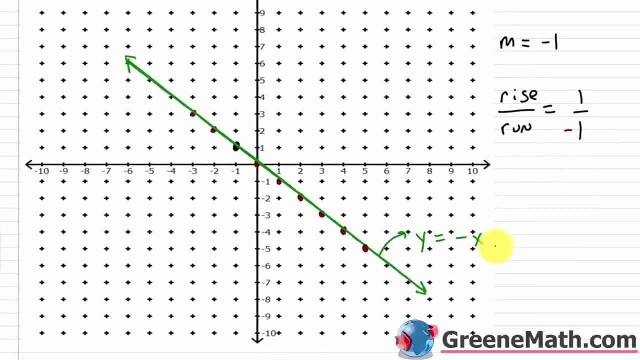 And later on we're going to learn how to take this information that we have and find the equation for the line. So this is actually y equals negative x. And I know that you don't know how to do that yet. That's okay. We're going to learn it very very soon in the future. So quickly I want to show you that if I switched which ordered pair I labeled as x sub 1 y sub 1 with the ordered pair I labeled as x sub 2 y sub 2 that it would make no difference and your slope would still be negative 1. 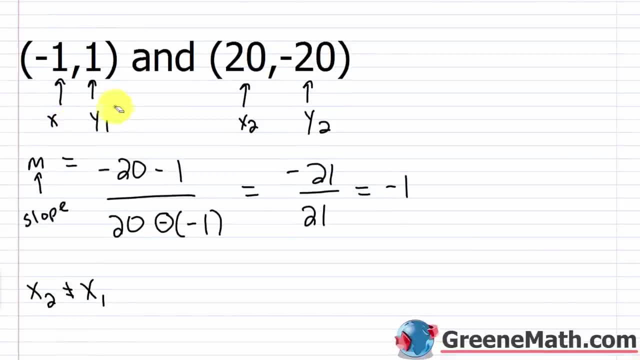 Let's do that real quick before we move on. Alright so let's just switch the way these are labeled. And so instead of this being x sub 1 y sub 1 it's going to be x sub 2 y sub 2. And this is going to be x sub 1 y sub 1. And let me erase this real quick. So the slope formula again it's m is equal to y sub 2 minus y sub 1 over x sub 2 minus x sub 1. 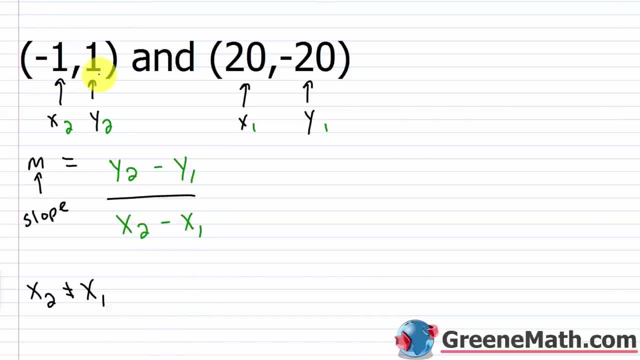 And let's just crank this out real quick. So y sub 2 is now 1. So I'm going to plug that in. And minus y sub 1 y sub 1 is negative 20. Again pay close attention. You're plugging in a negative 20. So that's going in there. And then this is over x sub 2 which is now negative 1 minus x sub 1 which is 20. 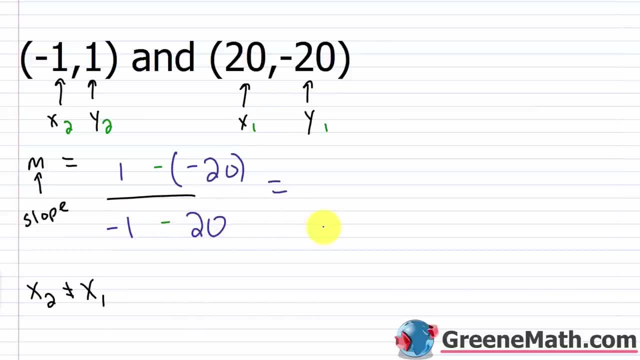 Minus 20. So what are we going to get? We have 1 minus a negative 20. That's the same thing as 1 plus 20. That's 21. 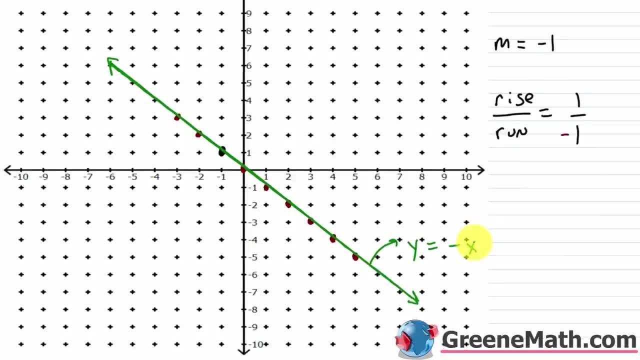 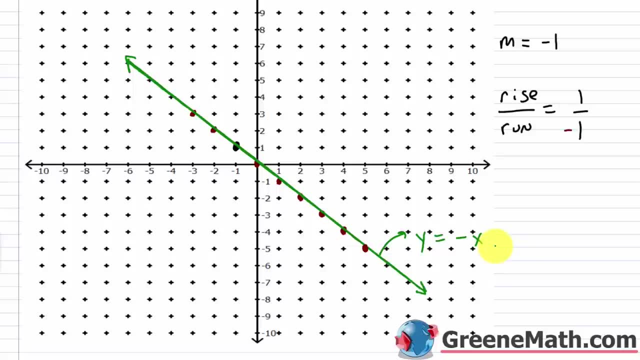 That's okay. We're going to learn it very, very soon in the future. So quickly I want to show you that if I switched which ordered pair I labeled as x sub 1, y sub 1 with the ordered pair I labeled as x sub 2, y sub 2, that it would make no difference. 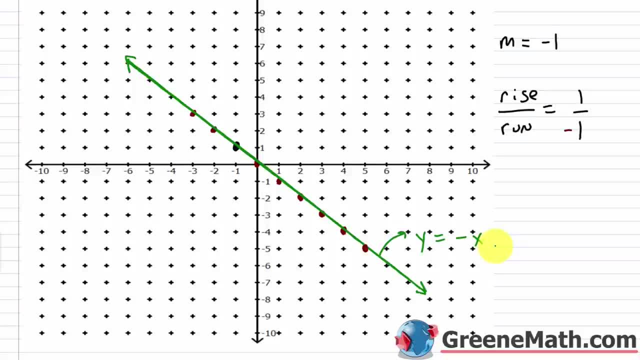 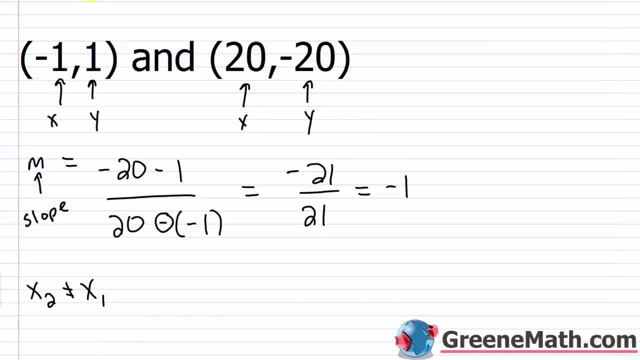 and your slope would still be negative 1.. Let's do that real quick before we move on. All right, So let's just switch the way these are labeled, And so, instead of this being x sub 1, y sub 1, it's going to be x sub 2, y sub 2.. 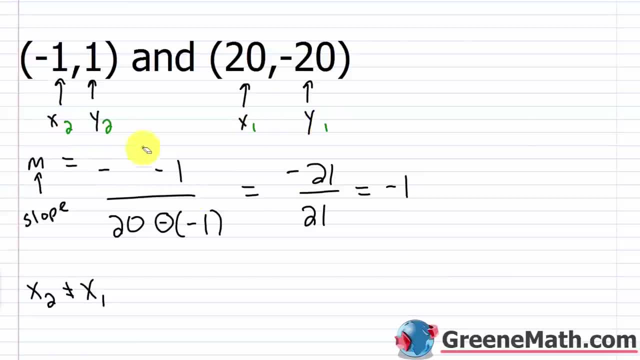 And this is going to be x sub 1, y sub 1.. And let me erase this real quick. So the slope formula again, it's m is equal to y sub 2 minus y sub 1 over x sub 2 minus x sub 1.. 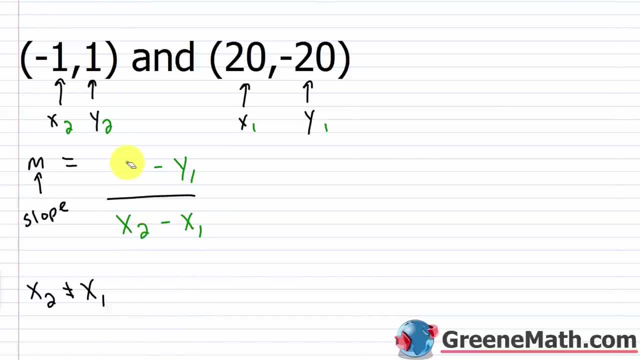 And let's just crank this out real quick. So y sub 2 is now 1.. So I'm going to plug that in And minus y sub 1, y sub 1 is negative 20.. Again, pay close attention. You're plugging in a negative 20.. 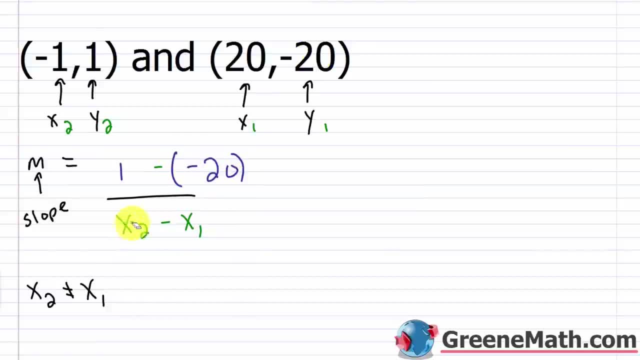 So that's going in there, And then this is over. We have x sub 2, which is now negative. 1 minus x sub 1, which is 20. Minus 20.. Okay, So what are we going to get? We have 1 minus a negative 20.. 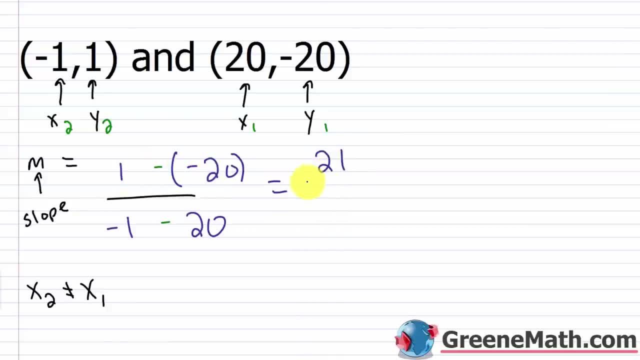 That's the same thing as 1 plus 20.. That's 21.. This is over. Here we have negative 1 minus 20, which is negative 21.. So again you see, it's going to be the same thing. 21 divided by negative 21 is negative 1.. 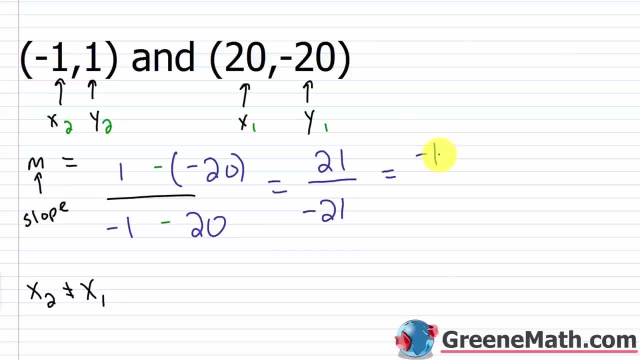 So this is negative 1.. Or again, in terms of slope, we could think about this as negative 1 over 1.. Or we could write it as 1 over negative 1.. Right again, as it relates to rise over run, we've already seen that we can use that in. 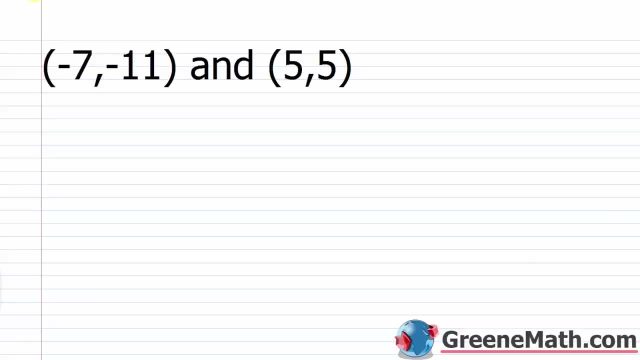 two different ways. All right, let's take a look at the next problem. So we have the ordered pair negative 7 comma negative 11 and 5 comma 5.. So these two points are what we're given And we want to calculate the slope. 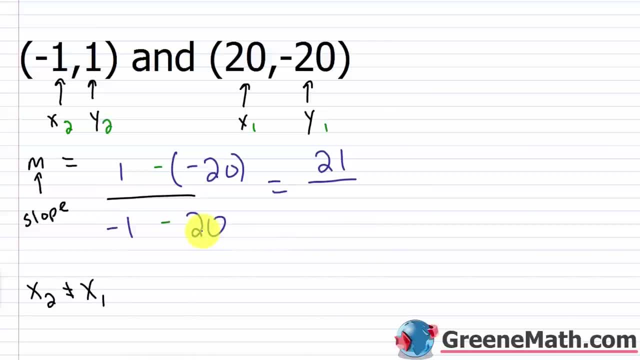 This is over. Here we have negative 1 minus 20 which is negative 21. So again you see it's going to be the same thing. 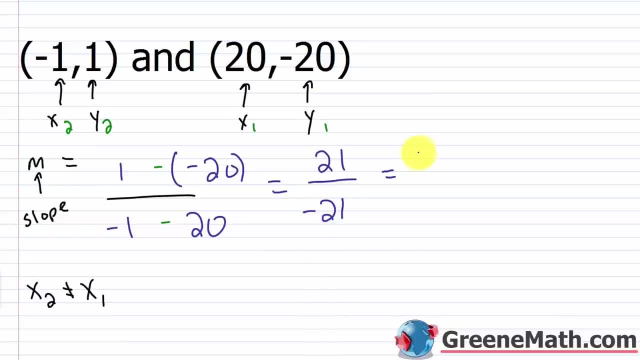 21 divided by negative 21 is negative 1. So this is negative 1. Or again in terms of slope we can think about this as negative 1 over 1. Or we could write it as 1 over negative 1. 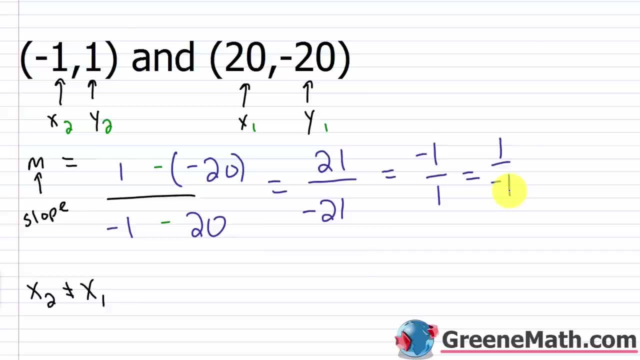 Again as it relates to rise over run we've already seen that we can use that in two different ways. Alright let's take a look at 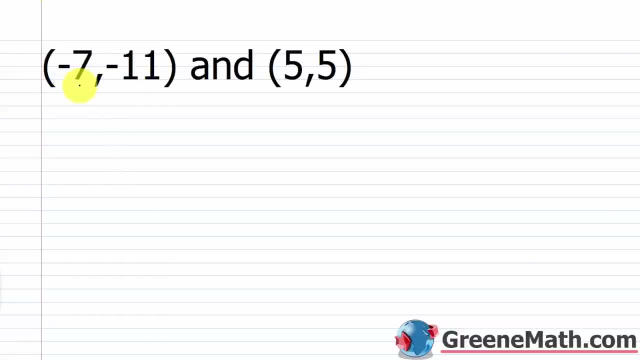 the next problem. So we have the ordered pair negative 7 comma negative 11 and 5 comma 5. So these two points are what we're given. And we want 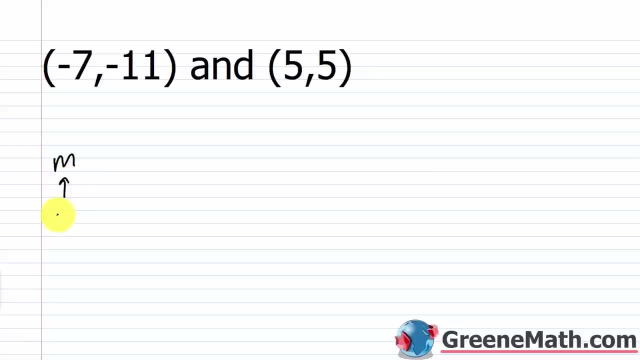 to calculate the slope. So m again our slope is equal to y sub 2 minus y sub 1 over x sub 2 minus x sub 1. 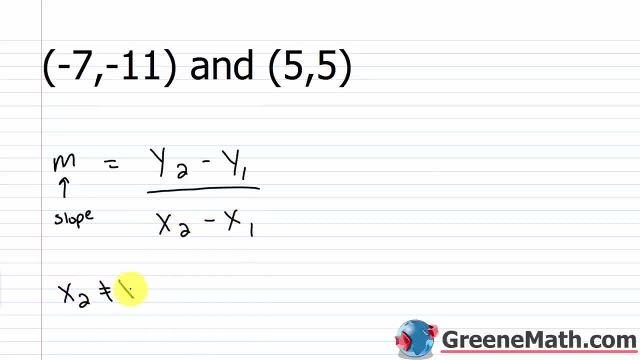 And again x sub 2 cannot be equal to x sub 1. 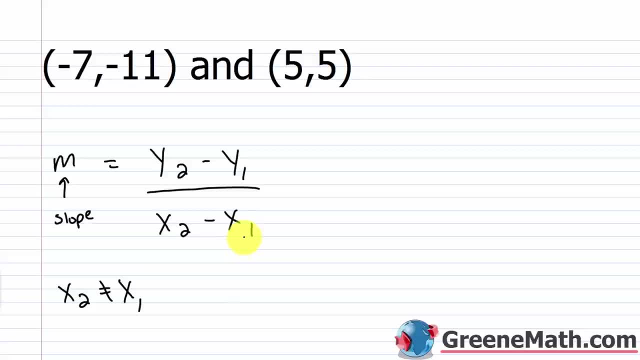 So we're going to label our points and a general practice for me and probably for you is just to label the first point as x sub 1 y sub 1. 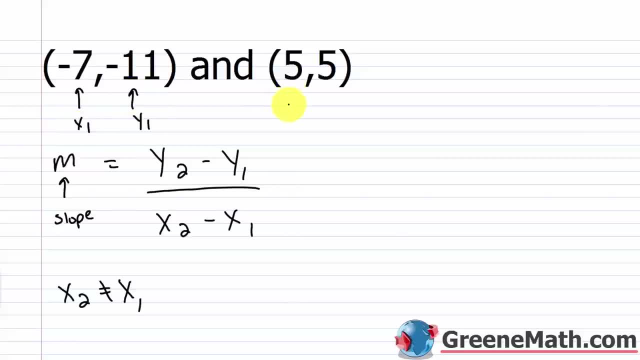 And again as I just showed you it doesn't matter. You get the same answer either way. And this one's going to be x sub 2 y sub 2. Okay. So y sub 2 is 5. So let me erase that and put a 5. 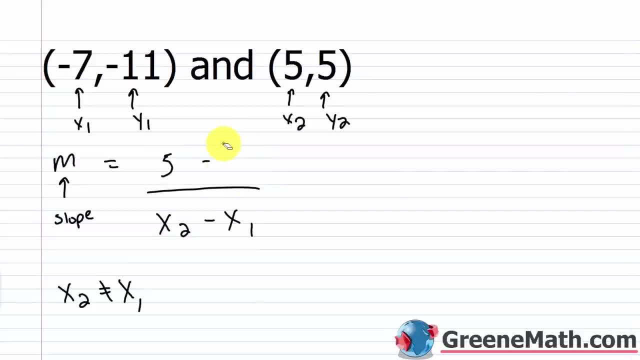 Minus y sub 1 that's negative 11. Let me erase this and put negative 11. This is over. We have x sub 2. 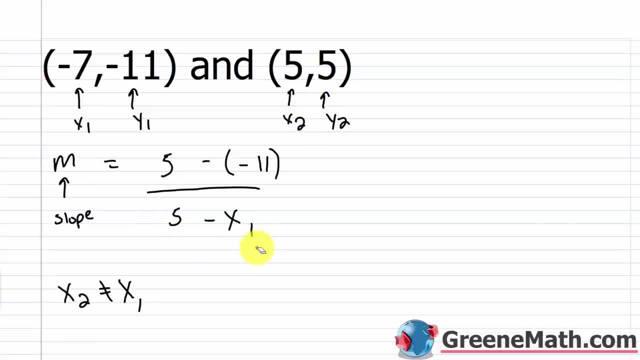 That's going to be 5. Minus x sub 1 which is negative 7. So minus and negative 7. So in each case here we have to pay close attention to our signs because we have minus and negative. So 5 minus and negative 11 is the same thing as 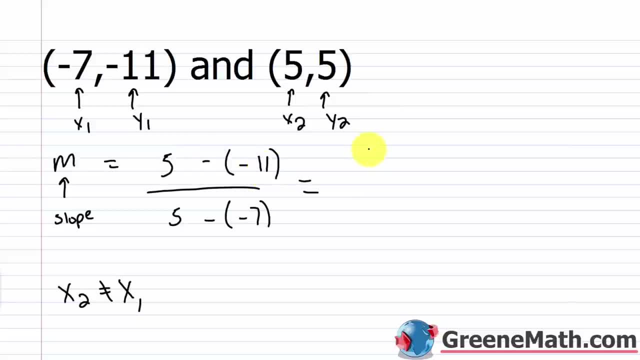 5 plus 11 which is 16. 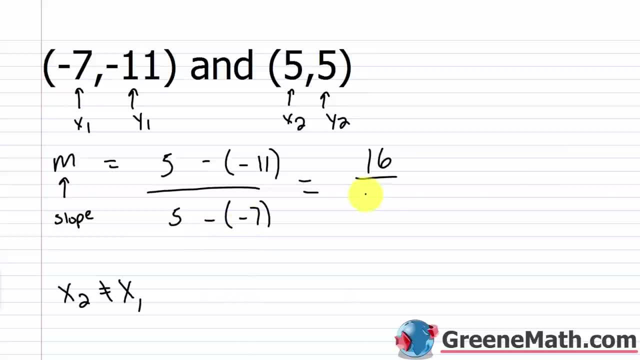 minus and negative 7 is the same thing as 5 plus 7 and that's 12. 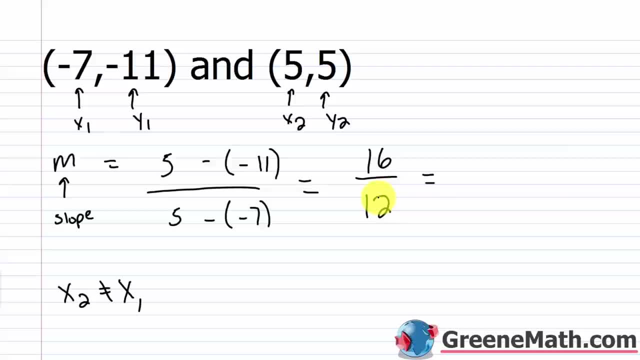 Now we can reduce this. Both are divisible by 4. 16 divided by 4 is 4. 12 divided by 4 is 3. 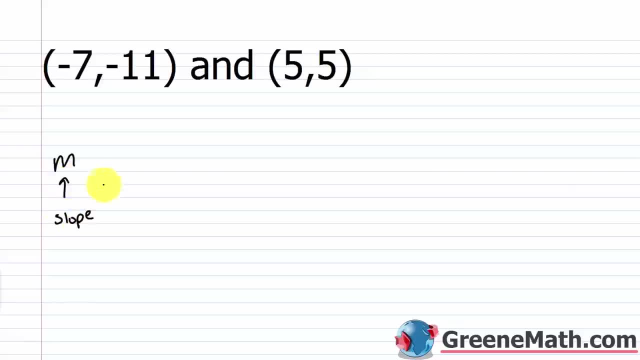 So m Again, The slope is equal to y sub 2 minus y sub 1 over x sub 2 minus x sub 1.. And again, x sub 2 cannot be equal to x sub 1.. So we're going to label our points. 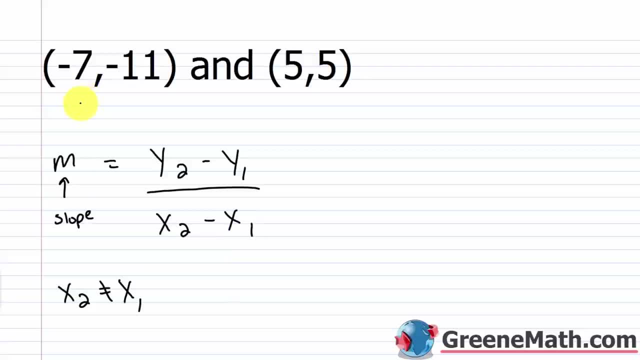 And a general practice for me and probably for you, is just to label the first point as x sub 1, y sub 1.. And again, as I just showed you, it doesn't matter, You get the same answer either way, And this one's going to be x sub 2, y sub 2.. 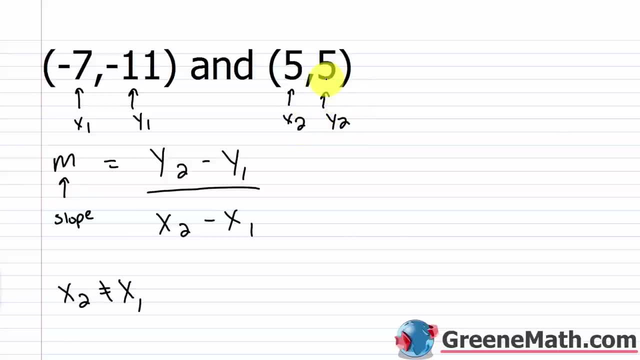 Okay, So y sub 2 is 5.. So let me erase that and put a 5. Minus y sub 1, that's negative 11.. Let me erase this and put negative 11.. This is over. We have x sub 2.. 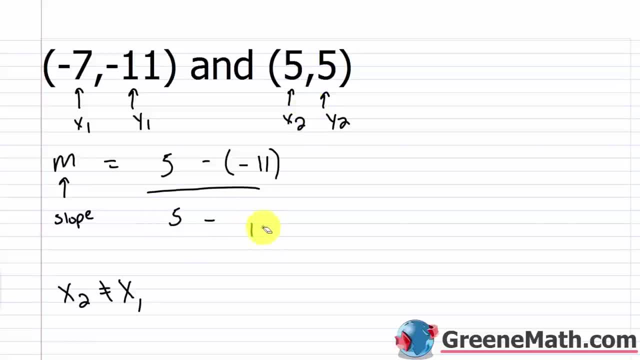 That's going to be 5. Minus x sub 1, which is negative 7. So minus a negative 7.. So in each case here we have to pay close attention to our signs, because we have minus and negative. So 5 minus a negative 11.. 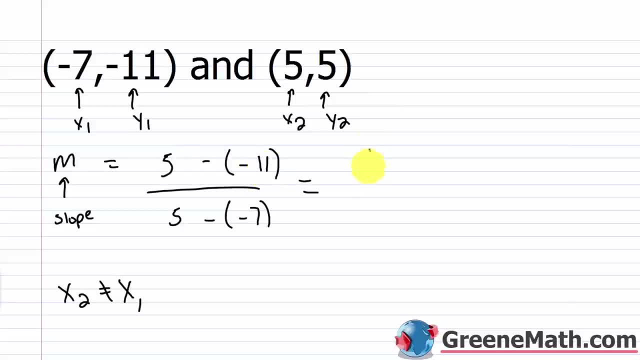 Is the same thing as 5 minus a negative 7.. So we're going to put negative 7.. 5 plus 11, which is 16.. 5 minus a negative 7 is the same thing as 5 plus 7, and that's 12.. 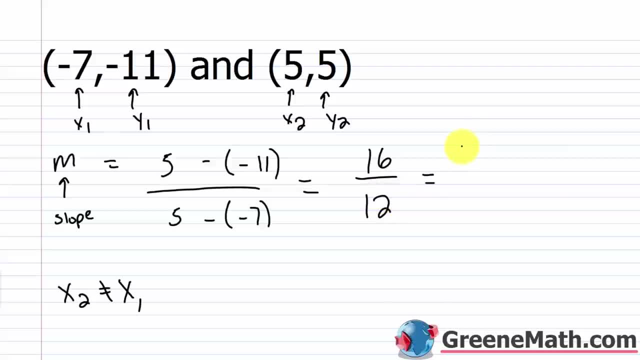 Now we can reduce this. Both are divisible by 4.. 16 divided by 4 is 4.. 12 divided by 4 is 3.. So we get 4 thirds here, or 4 over 3.. Now we think about this in terms of, again, rise over run. 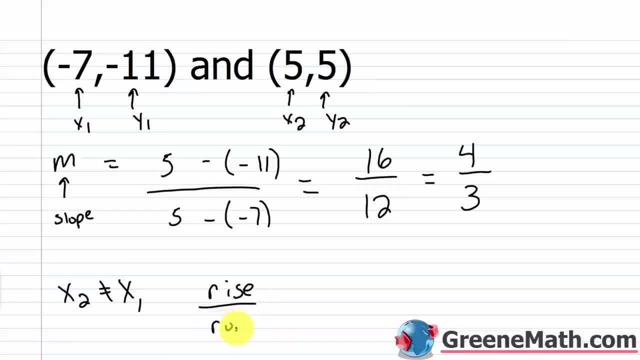 So rise over run is equal to 4 over 3.. So that means that If I'm at a given point on a line, I can rise 4 units or go up 4 units and then run 3.. So go to the right 3 and I'll end up at another point on that line. 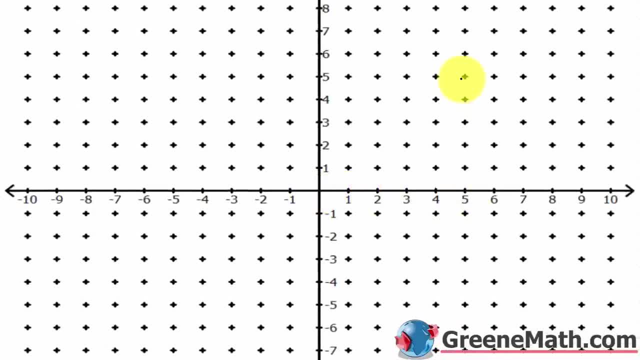 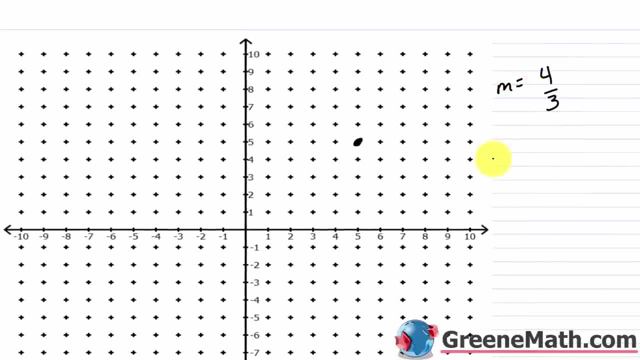 So a point on the line is 5 comma 5.. So that's going to be right. here Again, our slope M is equal to 4 thirds. So in terms of rise over run, This is 4 over 3.. So if I wanted to find another point on this line, 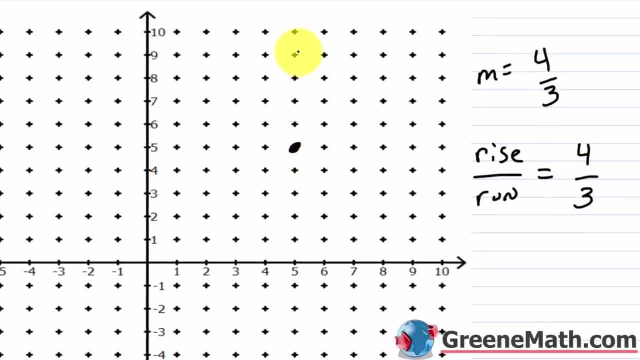 I could go up 4.. So up 1,, 2,, 3,, 4.. And then I could run 3.. When you talk about run, Again, positive means you go to the right. So I'm going to the right 3.. 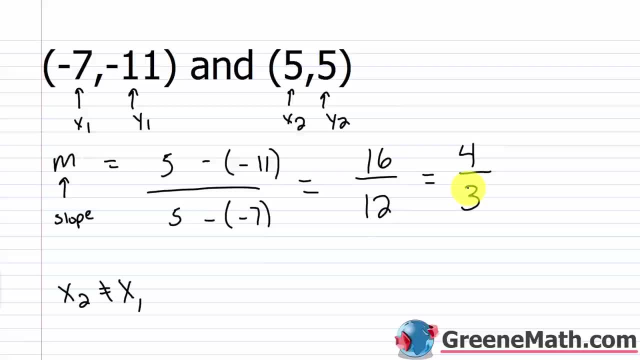 So we get 4 thirds here or 4 over 3. Now we 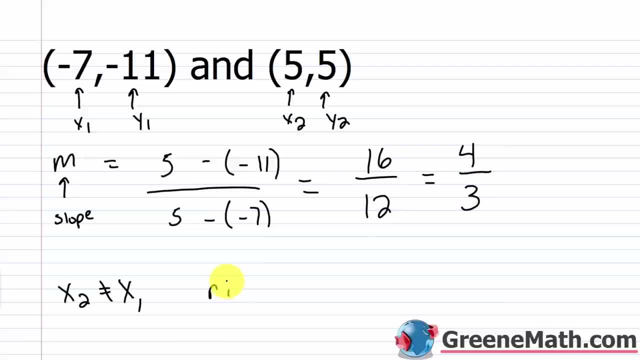 think about this in terms of again rise over run. So rise over run is equal to 4 over 3. So that means that if I'm at a given point on a line I can rise 4 units or go up 4 units and then run 3. So go to 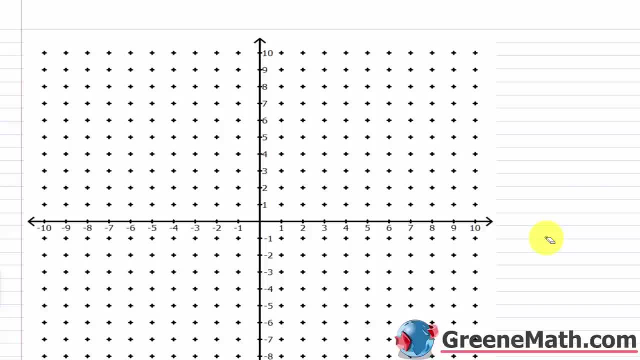 the right 3 and I'll end up at another point on that line. So a point on the line is 5 comma 5. So that's going to be right here. 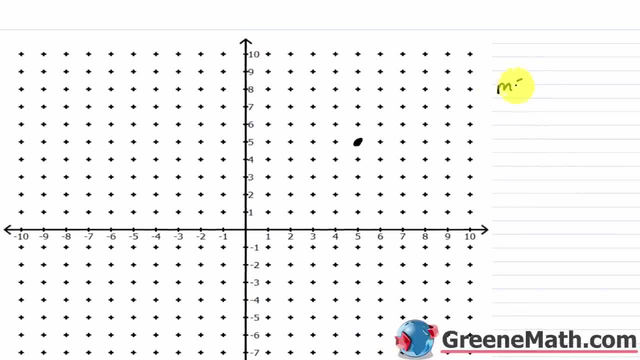 Again our slope m is equal to 4 thirds. 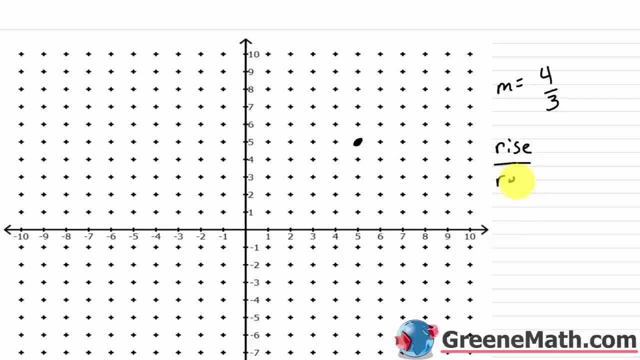 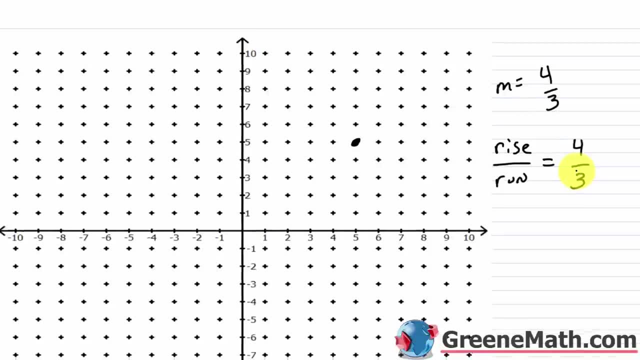 So in terms of rise over run this is 4 over 3. So if I wanted to find another point on this line I could go up 4. 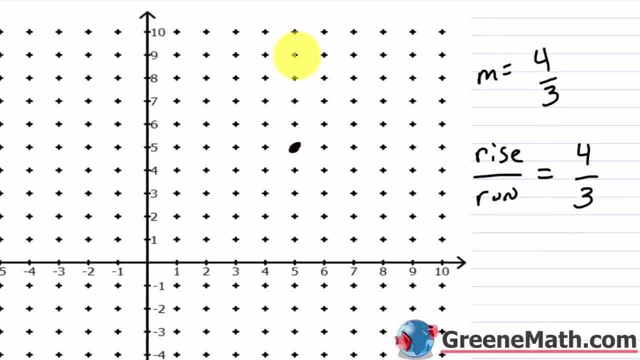 So up 1, 2, 3, 4 and then I could run 3. Okay when you talk about run 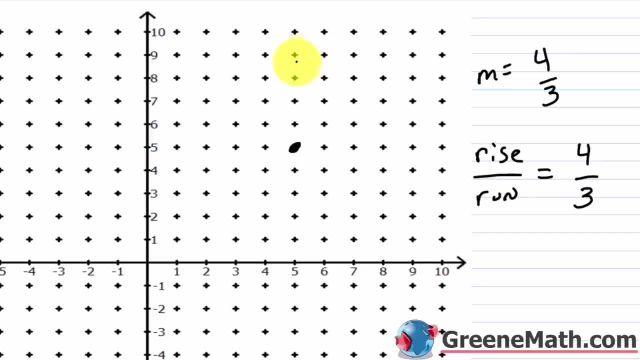 again positive means you go to the right. So I'm going to the right 3. 1, 2, 3. So here's another point on that line. 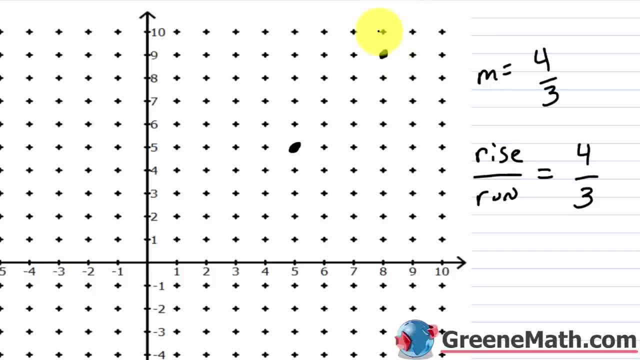 Now let's say you are out of space going up on your graph like I am. My kind of top number here is 10. 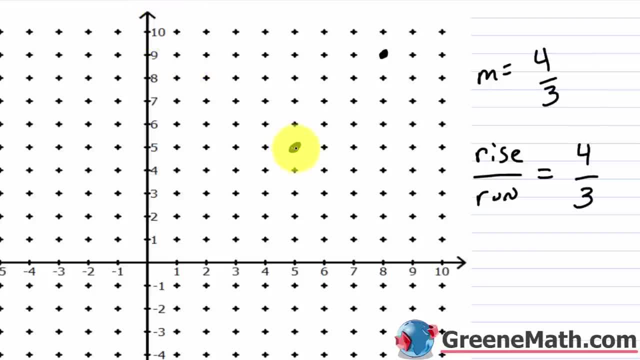 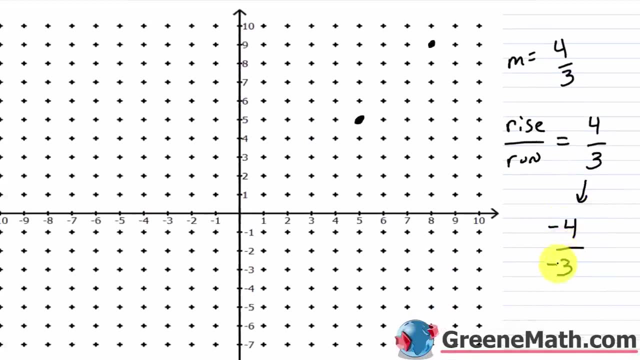 Well no problem. You could start at 5 comma 5 and you can go in this direction. You might say well how do you do that? Well one cool trick is to remember that a negative divided by a negative is a positive. So really I could write this as negative 4 over negative 3. This has the same mathematical value as 4 thirds because if I divide a negative by a negative I get a positive which is what I have here. 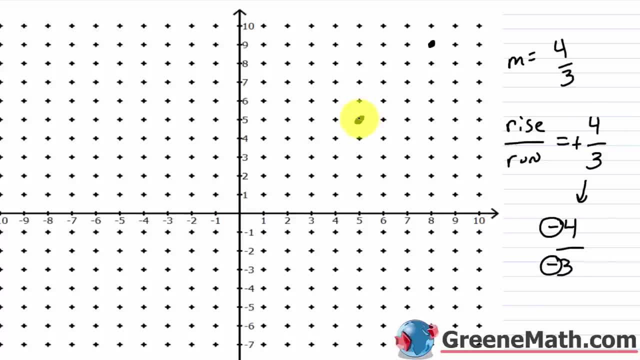 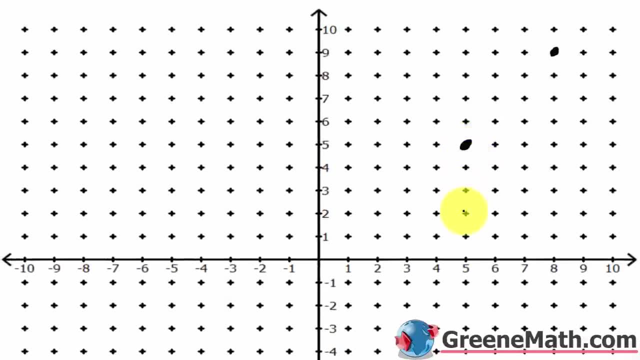 So using that thought process I could start at this point and I could fall 4 units. That's what negative 4 means in terms of rise. So I would go 1, 2, 3, 4. And then I could go to the left 3 units. That's what negative 3 means in terms of run. I'm going to the left. So 1, 2, and then 3. So here's another point on the line. And I could do that again. 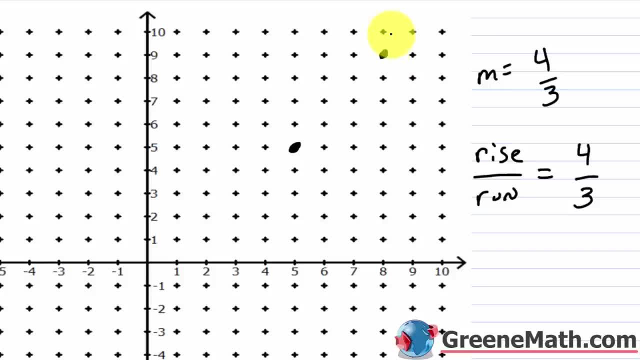 1,, 2,, 3.. So here's another point on that line. Now let's say you are out of space going up on your graph Like I am. My kind of top number here is 10.. Well, no problem. 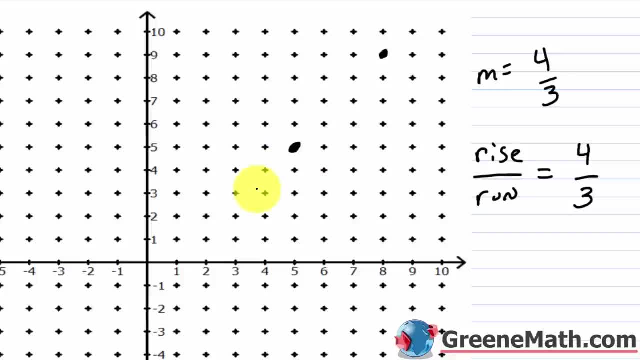 You could start at 5, comma 5.. And you can go in this direction. You might say: well, how do you do that? Well, one cool trick is to remember that a negative divided by a negative is a positive. So really I could write this as negative 4 over negative 3.. 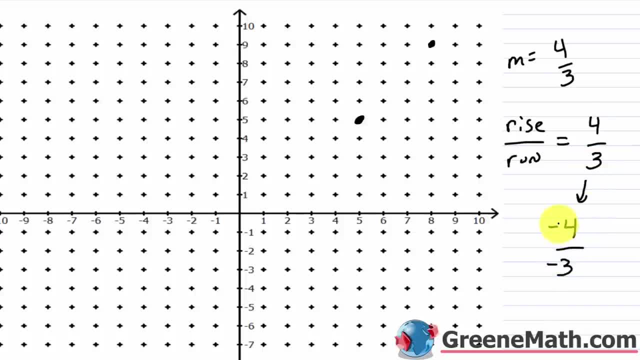 This has the same mathematical value as 4 thirds, because if I divide a negative by a negative, I get a positive, Which is what I have here. So, using that thought process, I could start at this point and I could fall 4 units Right. 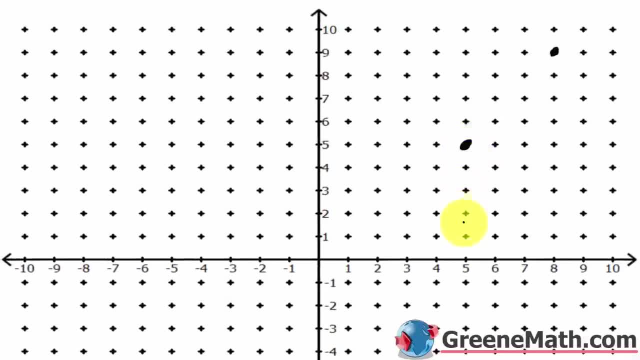 That's what negative 4 means in terms of rise. So I would go 1,, 2,, 3,, 4. And then I could go to the left 3 units. That's what negative 3 means in terms of run. 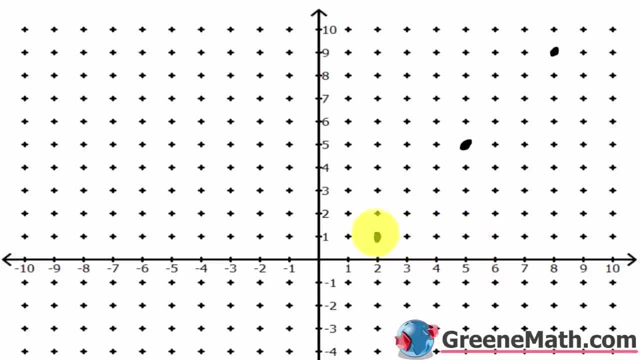 Right, I'm going to the left. So 1,, 2, and then 3.. So here's another point on the line And I could do that again. I'm going to fall 4.. 1,, 2,, 3,, 4.. 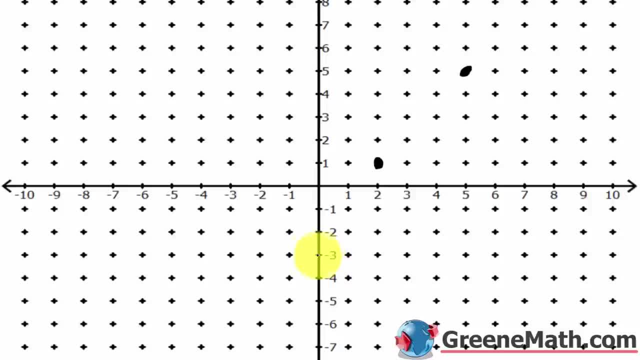 I'm going to run to the left- 3.. 1,, 2,, 3.. So here's that, And then I could graph this line if I wanted to. I'm going to run to the left- 3.. 1,, 2,, 3.. 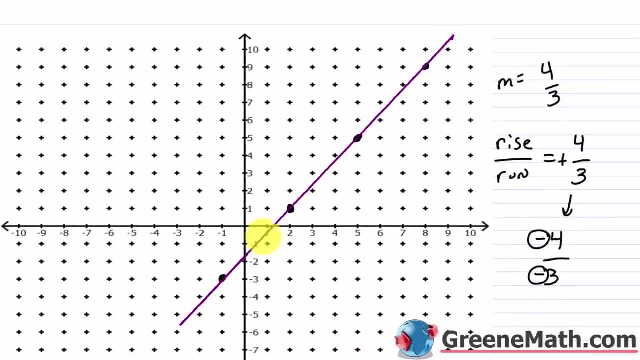 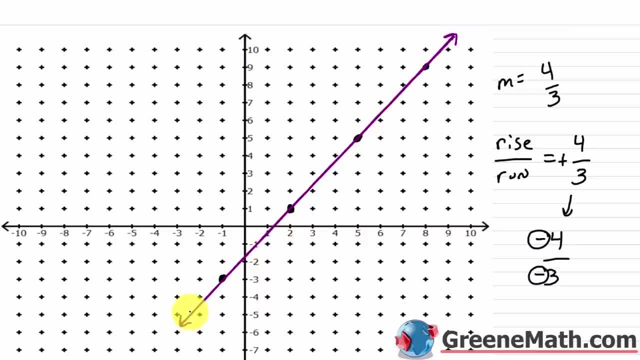 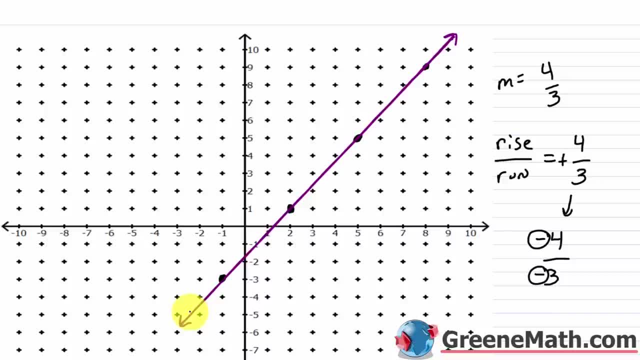 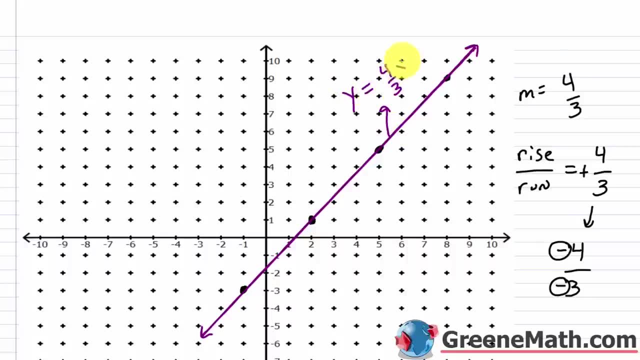 Again. I know that you don't know how to figure that out yet, But I'm just going to go ahead and give it to you, And so this would be the graph, for Y equals 4 thirds, X minus 5 thirds, And again, really shortly we're going to learn how to do that. 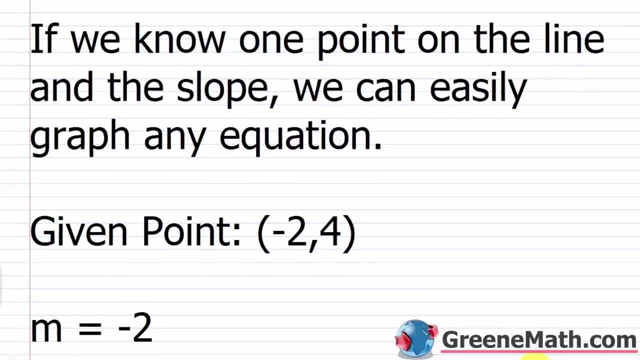 Alright. So, as you may or may not have figured out at this point, If you know one point on the line and the slope, we can easily graph any equation. This is kind of the preferred method to do it. You saw kind of in the last lesson where we go through and make these ordered pairs and 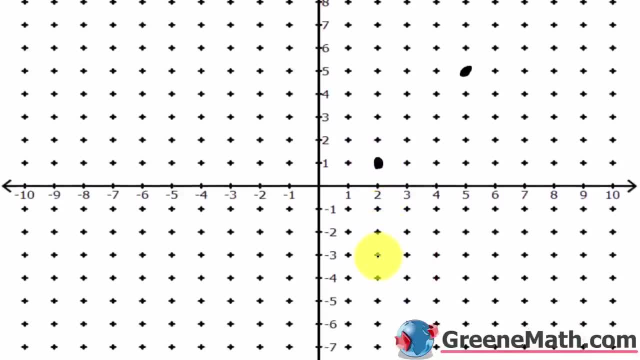 I'm going to fall 4. 1, 2, 3, 4. I'm going to run to the left 3. 1, 2, 3. 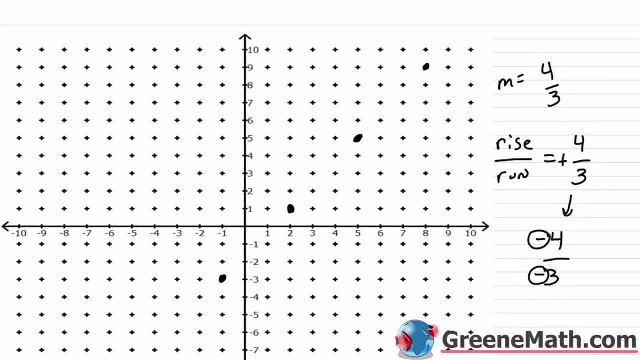 So here's that. And then I could graph this line if I wanted to. 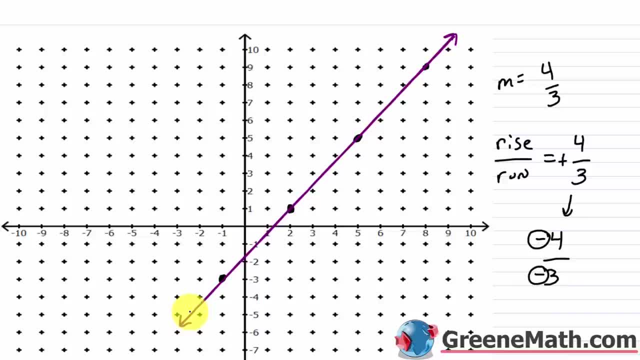 And again not perfect but kind of the best I can do. Alright. And then what's the equation 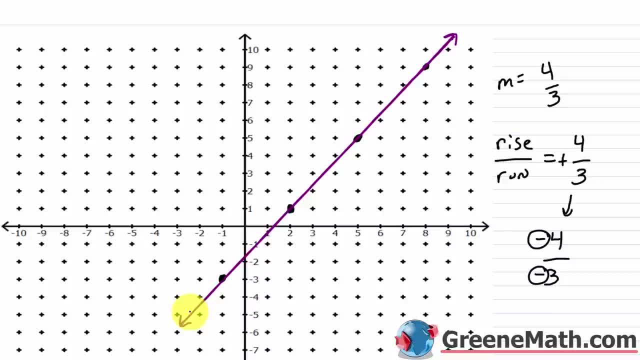 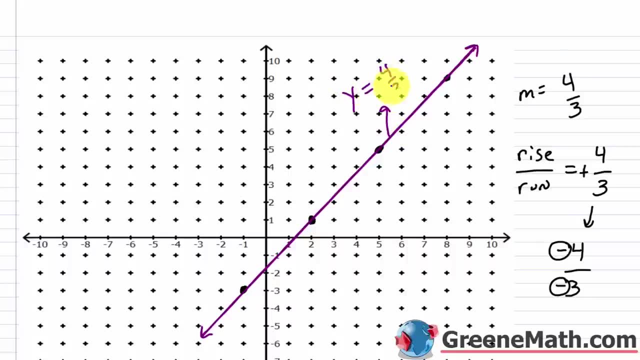 for this line? Again I know that you don't know how to figure that out yet. But I'm just going to go ahead and give it to you. And so this would be the graph for y equals 4 thirds x minus 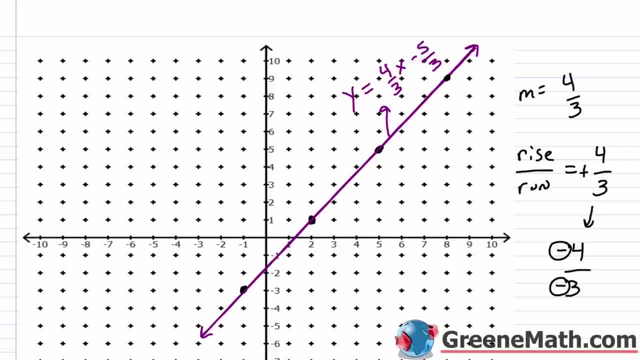 5 thirds. And again really shortly we're going to 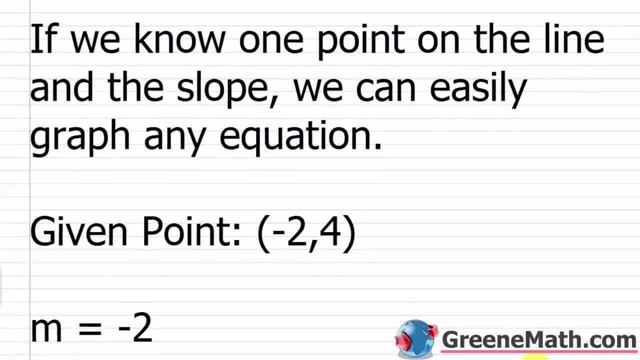 learn how to do that. Alright so as you may or may not have figured out at this point. If you know one point on the line and the slope we can easily graph any equation. And this is kind of the preferred method to do it. You saw kind of in the last lesson where we go through and make these ordered pairs. And even though with the intercept method it's a little bit easier. 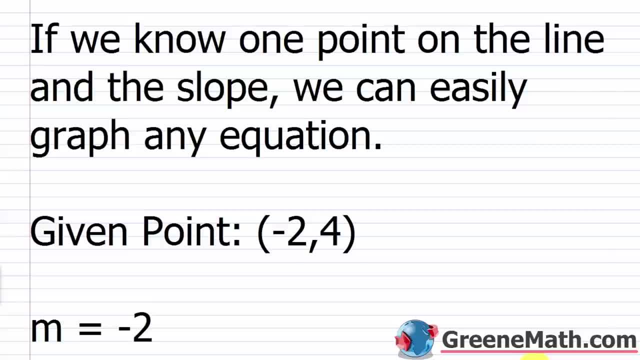 This method of graphing is just so so fast. So 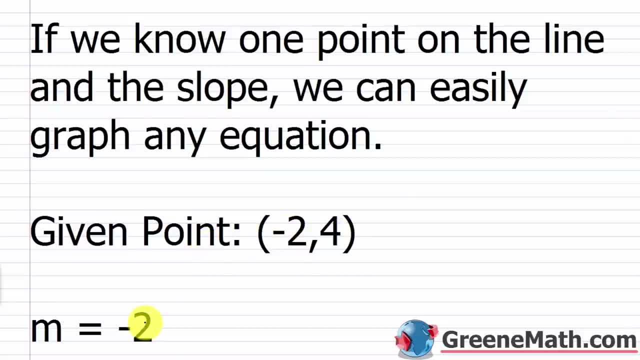 my given point is negative 2 comma 4 and my slope is negative 2. So again m is negative 2 and my given point is negative 2 comma 4. 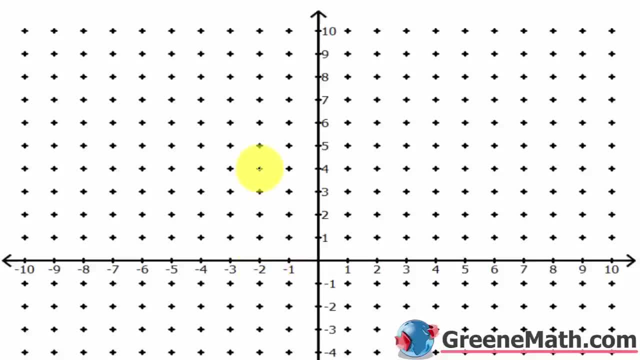 So here's negative 2. Here's 4. 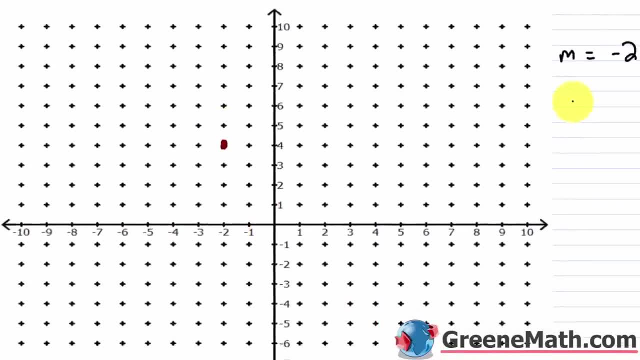 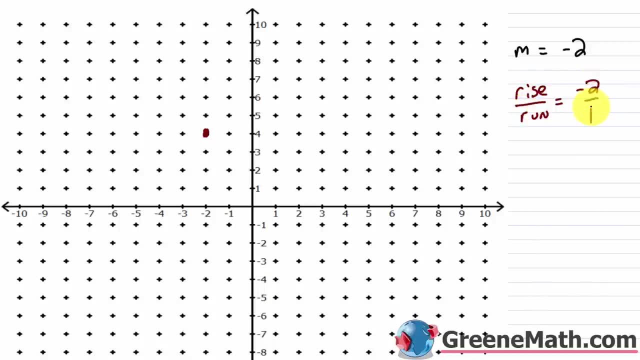 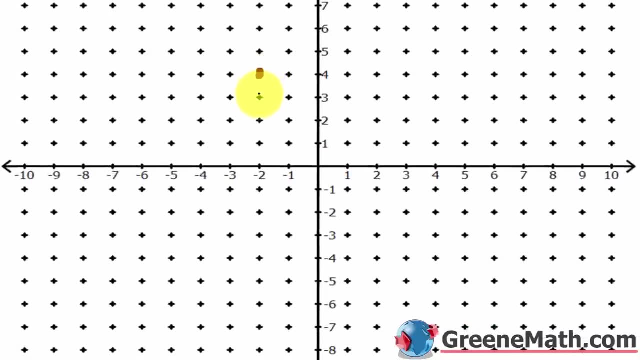 So that would be negative 2 comma 4. And if my slope is negative 2 again that means that my rise over run is equal to negative 2 over 1. So that means I'm falling 2 units for every 1 unit I go to the right. So starting here I would go 1 2 down and then 1 to the right. 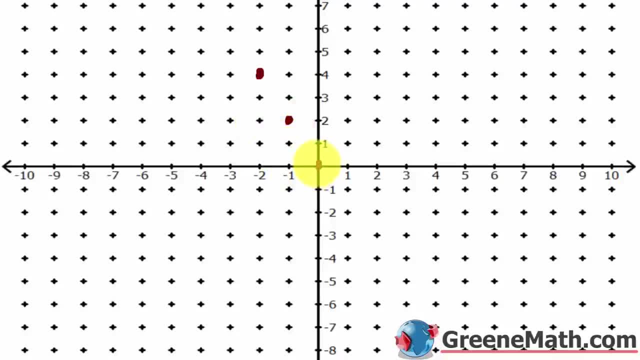 There's a point. 1 2 down and 1 to the right. There's a point. And once you have 3 points. Really 2 you can draw the line. But 3 again is nice to get a nice clean line. And I like to do a few more actually if I'm free hand. 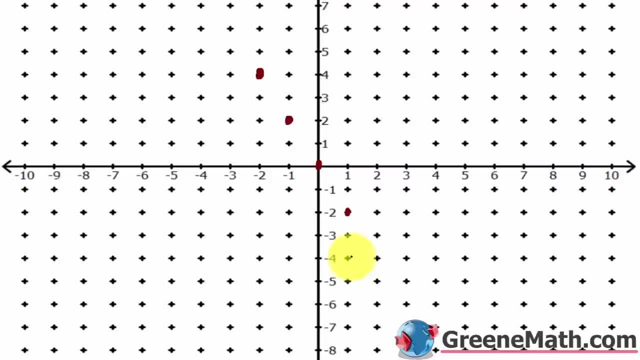 So 1 2 down 1 over. 1 2 down 1 over to the right. 1 2 down 1 over to the right. 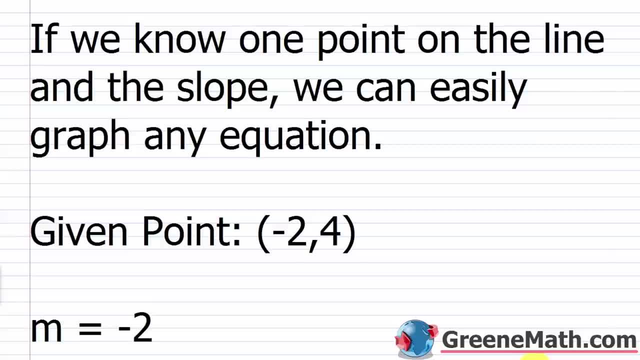 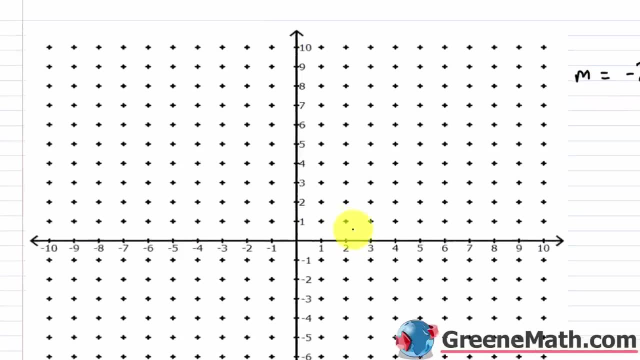 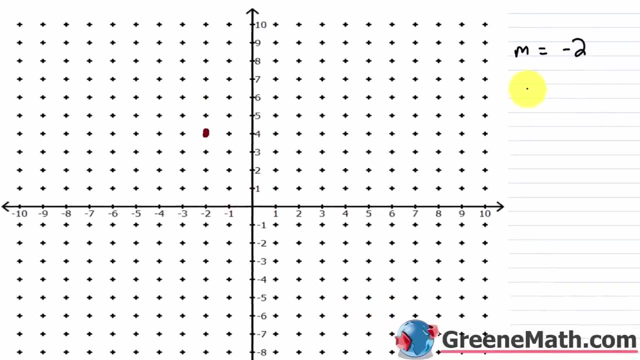 even though with the intercept method it's a little bit easier. this method of graphing is just so, so fast. So my given point is, and my slope is, So again, M is and my given point is: So here's, here's, 4, so that would be, and if my slope is again that: 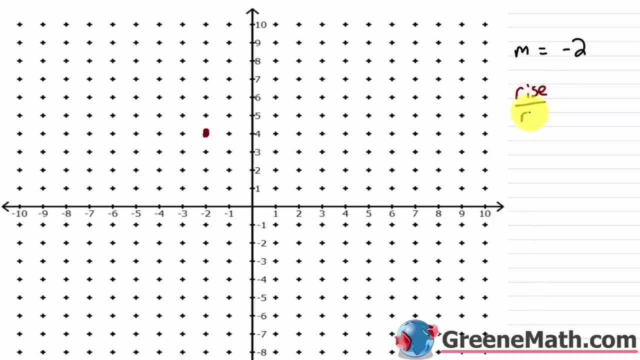 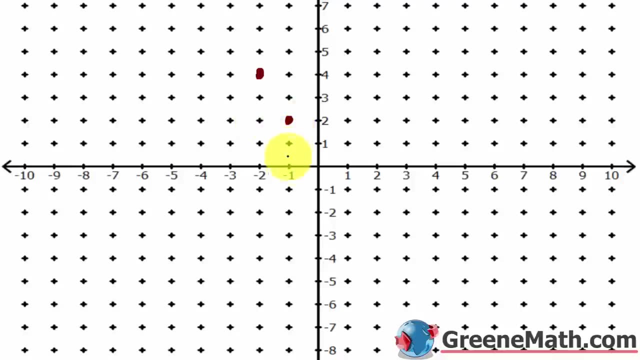 means that my rise over run is equal to. So that means I'm falling two units for every one unit I go to the right. So, starting here, I would go down and then to the right. There's a point: 1,, 2, down and 1 to the right. 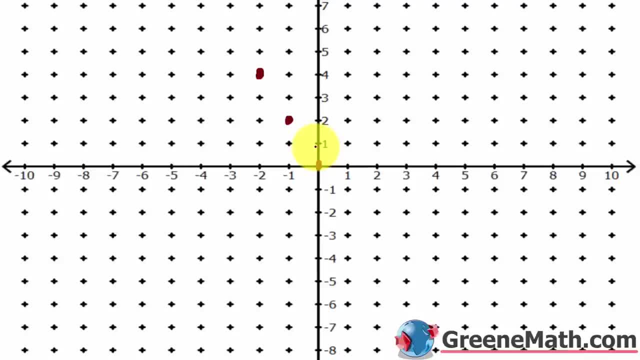 There's a point, And once you have three points- really two- you can draw the line right. but three again is nice to get a nice clean line and I like to do a few more actually from free hand. so 1, 2, down, 1, over. 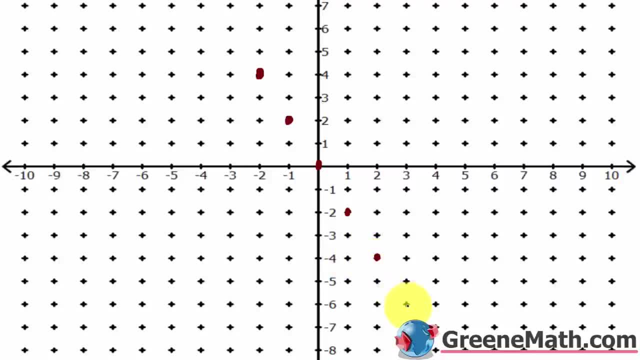 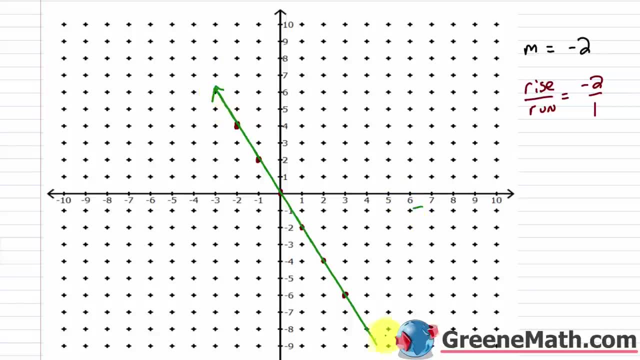 1, 2, down, 1, over to the right, 1, 2, down, 1, over to the right. So a faster way to graph a line. Okay, so another thing we want to talk about. let's say, you get. 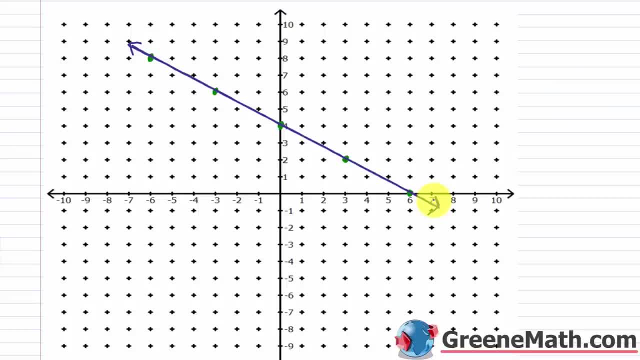 to your homework and you're presented with a graph, And so the graph of this line. they have some clearly indicated points and it asks for the slope of the line. Well, using the rise over run kind of thought process, so rise over run, you can calculate it. So let's say you start at one. 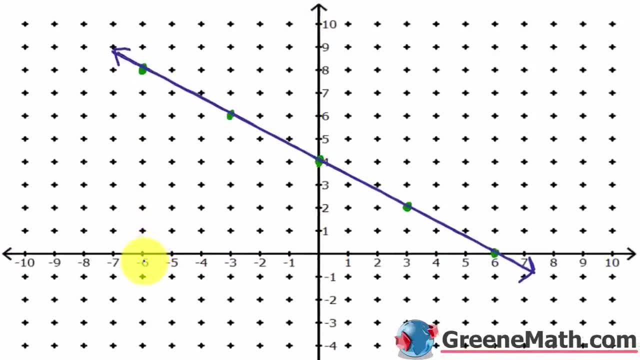 of the points. So this point right here looks like negative six comma eight. So negative six comma eight, All right. So you think what would I need to do to get to the next point? So how much do I rise? So to get over here I've got to fall right. So I'm rising by a negative amount, I'm going down. 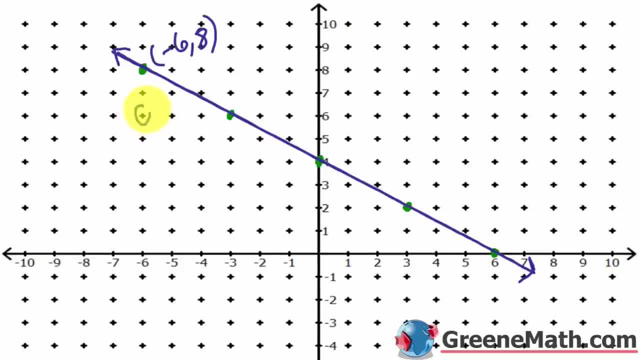 one, two units. So right here is not the next point, but it's the same Y location as the next point. So that means I'm falling. So I'm going down one, two units. So I'm going down one, two. 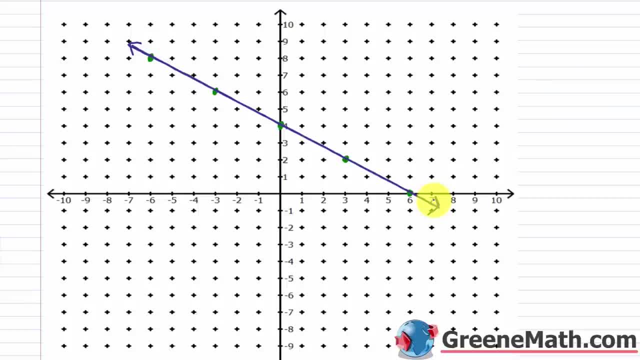 So kind of a faster way to graph a line. Okay so another thing we want to talk about. Let's say you get to your homework and you're presented with a graph. And so the graph of this line have some clearly indicated points and it asks for the slope of the line. Well using the rise over run kind of thought process. So rise over run. 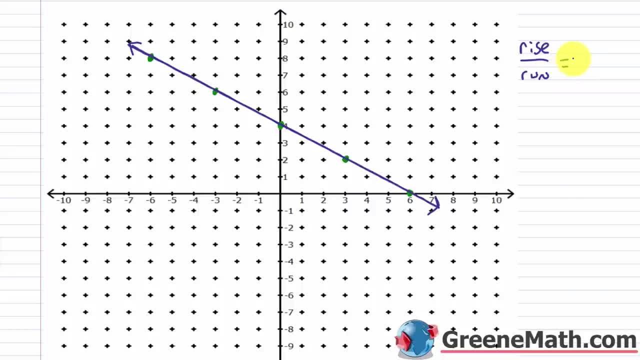 You can calculate it. So let's say you start at one of the points. 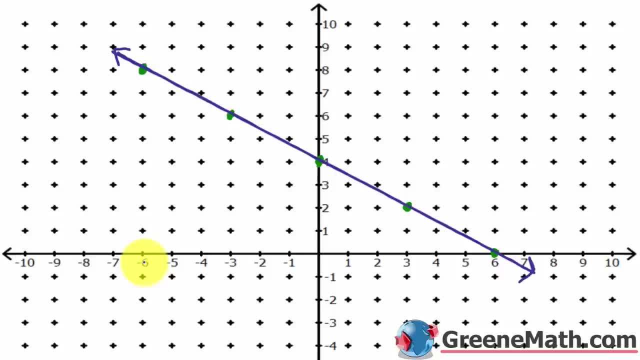 So this point right here looks like negative 6 comma 8. So negative 6 comma 8. 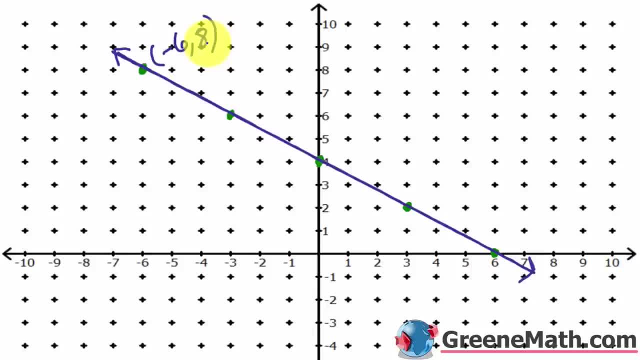 Alright. So you think what would I need to do to get to the next point. So how much do I rise. So to get over here I've got to fall. Right so I'm rising by a negative amount. I'm going down 1 2 units. So right here is not the next point. 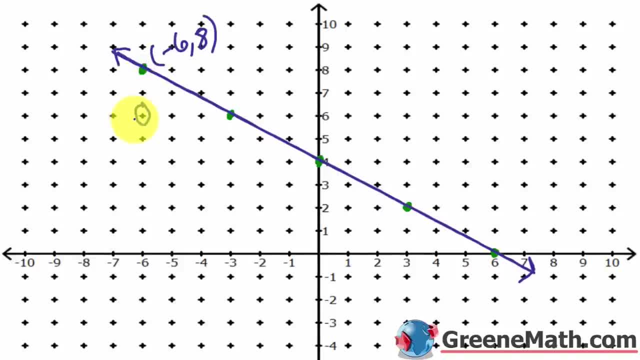 But it's the same Y location as the next point. So that means I'm falling by 2 units. 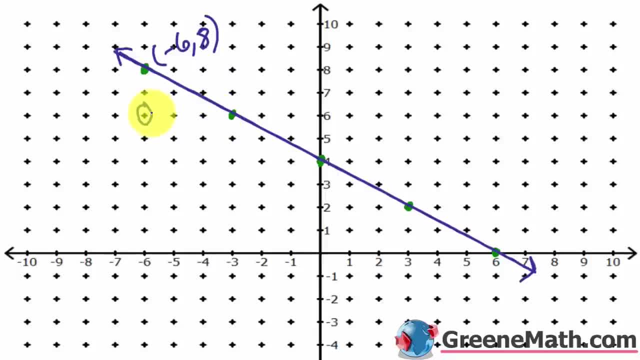 And then I'm running over to the right. Which is positive. I'm going over 1 2 3 units to the right. 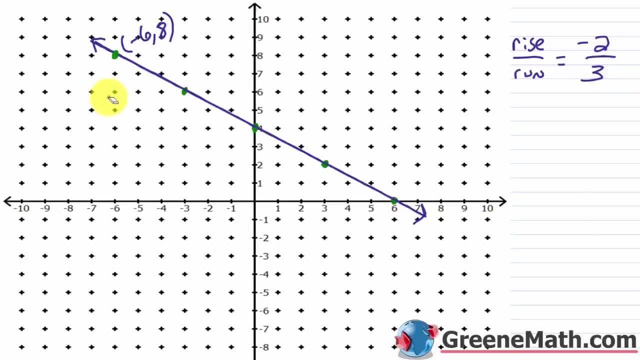 So my slope is negative 2 thirds. And then you can check that again starting at the next point. Down 2. 1 2. Go over to the right 3. 1 2 3. And I'm at the next point. 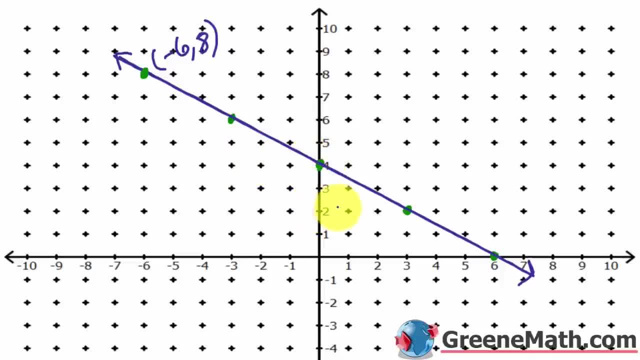 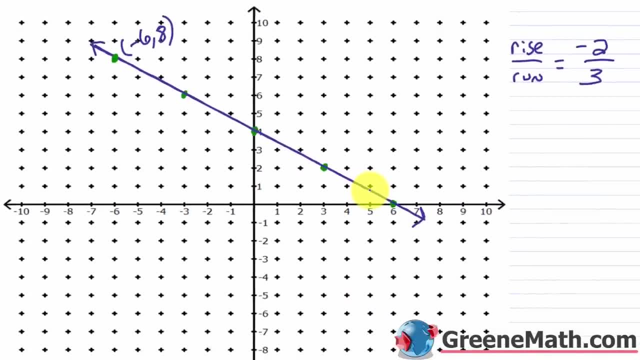 Down 2. 1 2. Over to the right 3. 1 2 3. I'm at the next point. Again you can keep doing that. So our slope in this case is negative 2 thirds. And then one of the other ways you could check this. You could look at one of the other points. So this point right here is negative 3 comma 6. So negative 3 comma 6. And you could use your slope formula and see if you get a slope of negative 2 thirds. So let's do that real quick. 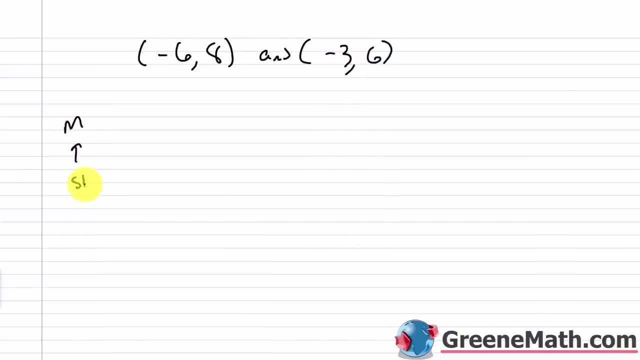 So remember your slope formula M. M is the slope. This is equal to Y sub 2 minus Y sub 1 over X sub 2 minus X sub 1. Again where X sub 2 does not equal X sub 1. And I'm just going to go ahead and label this first point as X sub 1 Y sub 1. And the second one as X sub 2 Y sub 2. 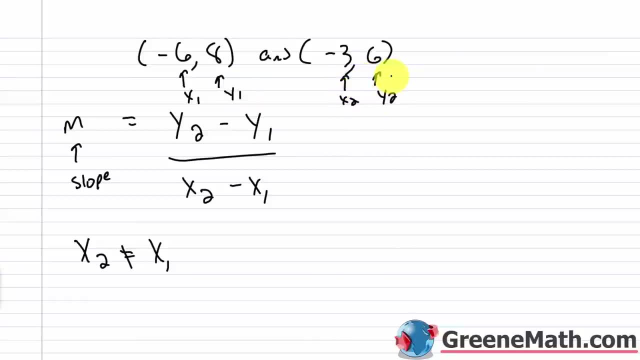 And again if you wanted to change that around you get the same answer. 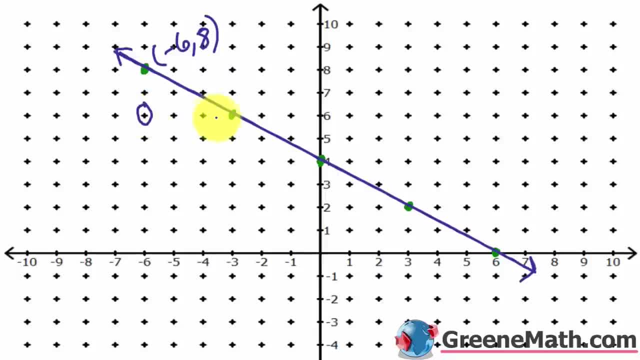 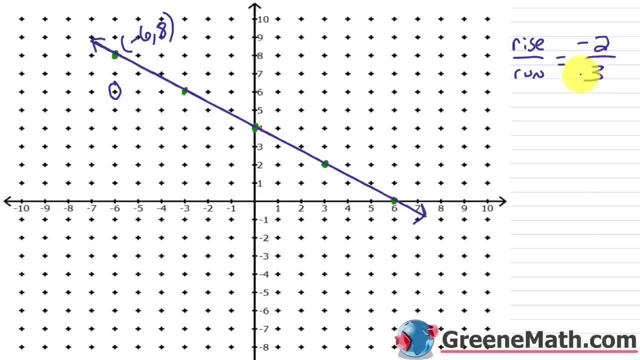 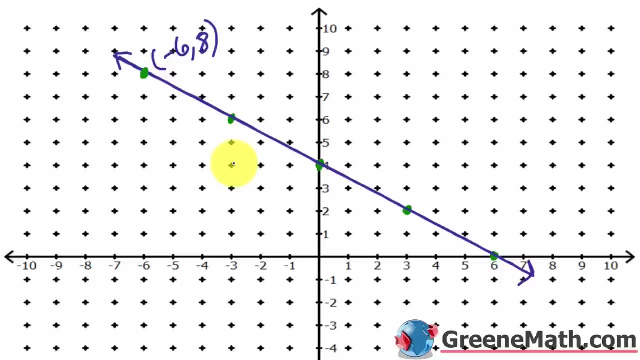 units. So I'm falling by two units And then I'm running over to the right, which is positive. I'm going over one, two, three units to the right. So my slope is negative, two thirds. And then you can check that again, starting at the next point: Down two, one, two, go over to the right, three. 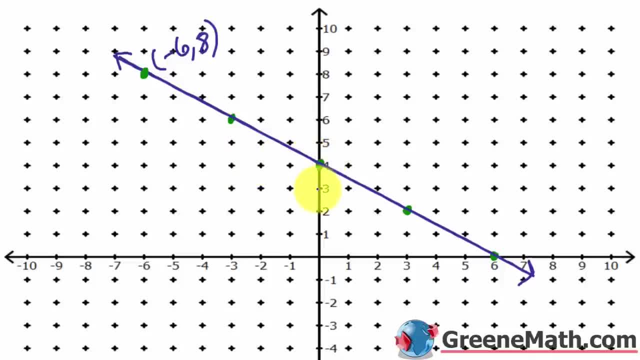 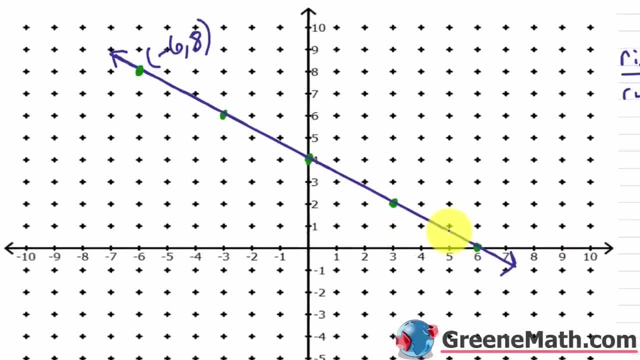 one, two, three- and I'm at the next point- Down, two, one, two, over to the right: three, one, two, three. I'm at the next point Again. you can keep doing that. So our slope in this. 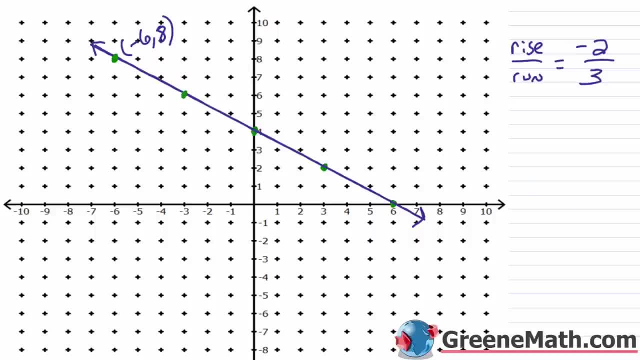 case is negative two thirds. So I'm going down one, two, three and I'm at the next point, two-thirds. and then one of the other ways you could check this, you could look at one of the other points. so this point right here is negative three comma six. 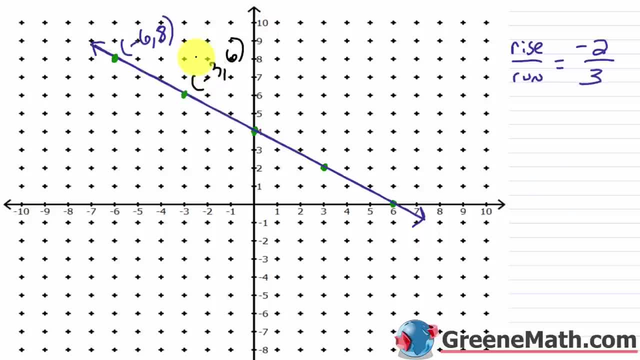 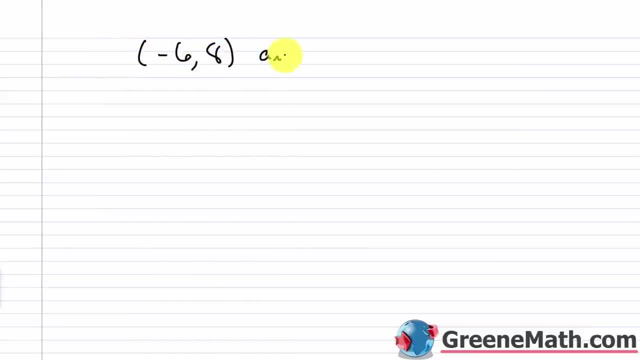 so negative three comma six and you could use your slope formula and see if you get a slope of negative two-thirds. so let's do that real quick. so remember your slope formula M and is the slope? this is equal to y sub 2 minus y sub 1 over x sub 2 minus x sub 1. again where x sub 2 does not equal x sub 1. 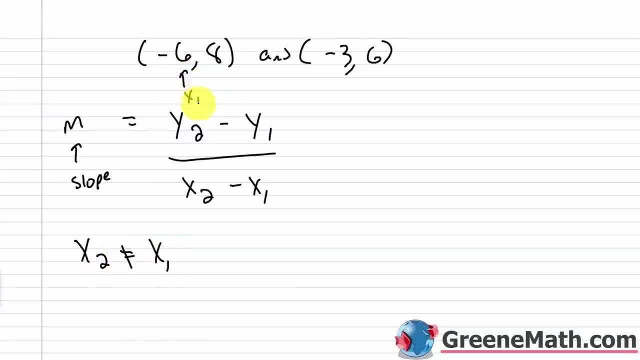 I'm just gonna go ahead and label this first point as x sub 1, y sub 1, and the second one as x sub 2, y sub 2, and again, if you wanted to change that around, you get the same answer. so y sub 2 is 6, so I'm gonna erase this and put a 6, y sub 1. 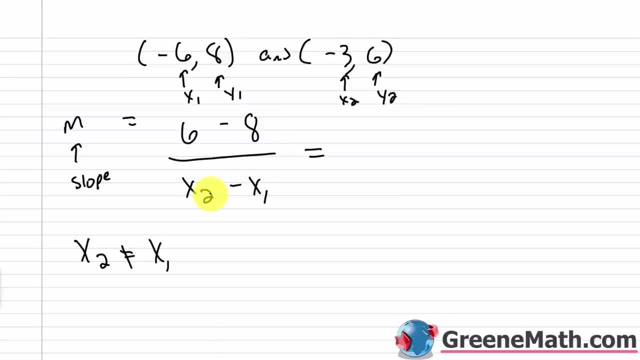 is 8, I'm gonna erase this and put an 8. x sub 2 is negative 3, so I'll erase this, put negative 3. and x sub 1 is negative 6, so I'm gonna erase this and put minus negative 6. or you can just do this right now and just say this is plus 6, so 6. 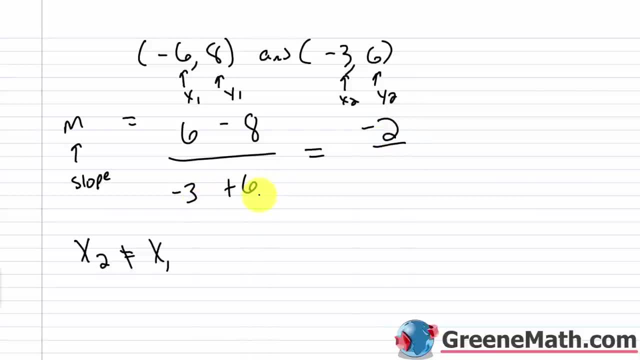 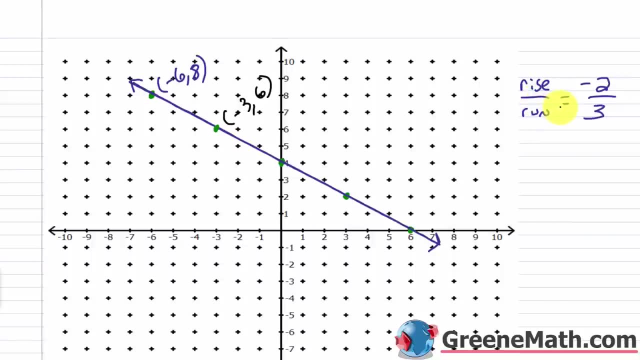 minus 8 is negative 2 and negative 3 plus 6 is 3, so you get negative 2 thirds at your slope and again that's exactly what you calculated here. your rise over 1 is equal to negative 2 thirds, or negative 2 over 3, all right. so now that 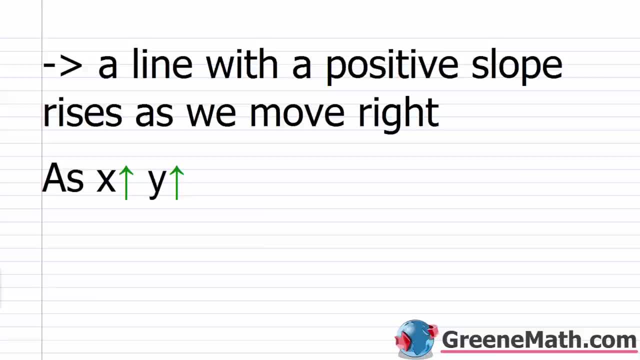 we have the basics down. let's wrap up our lesson with a few basic things that we need to keep in mind as we move to the right. so the first thing is that a line with a positive slope rises as we move to the right. so that kind of looks. 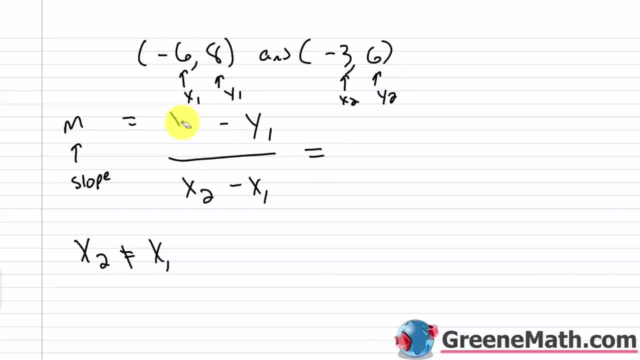 So Y sub 2 is 6. So I'm going to erase this and put a 6. Y sub 1 is 8. I'm going to erase this and put an 8. 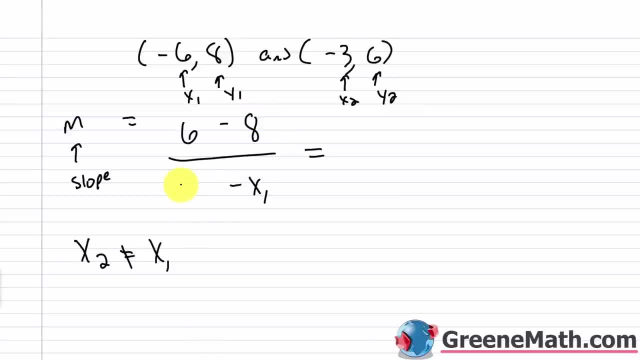 X sub 2 is negative 3. So I'll erase this and put negative 3. 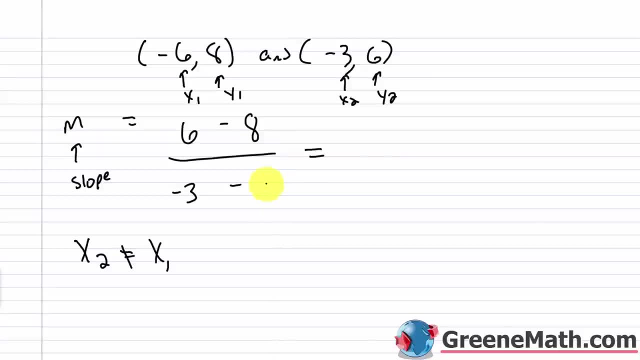 And X sub 1 is negative 6. So I'm going to erase this and put 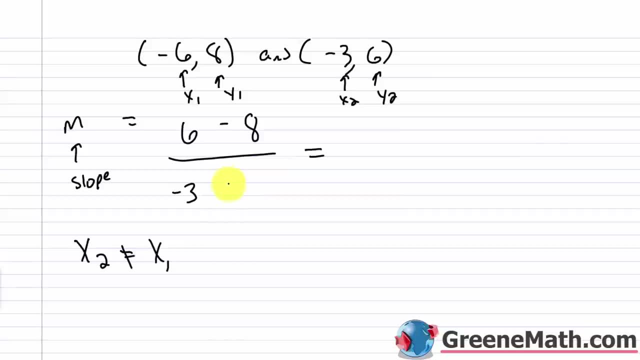 minus negative 6. Or you can just do this right now and just say this is plus 6. 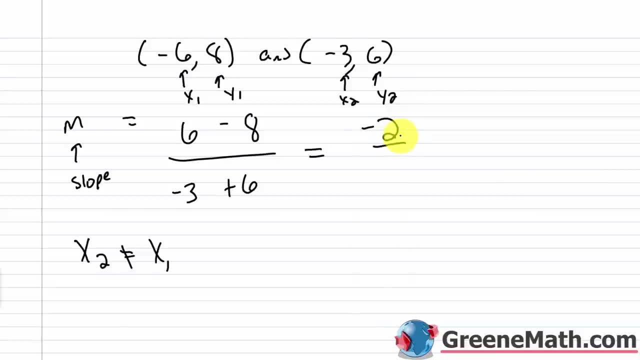 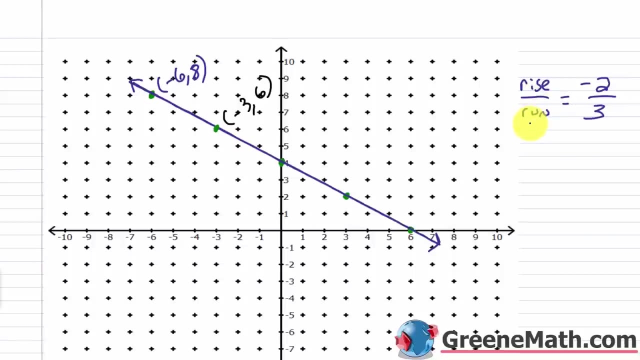 So 6 minus 8 is negative 2. And negative 3 plus 6 is 3. So you get negative 2 thirds as your slope. And again that's exactly what you calculated here. Your rise over 1 is equal to negative 2 thirds or negative 2 over 3. 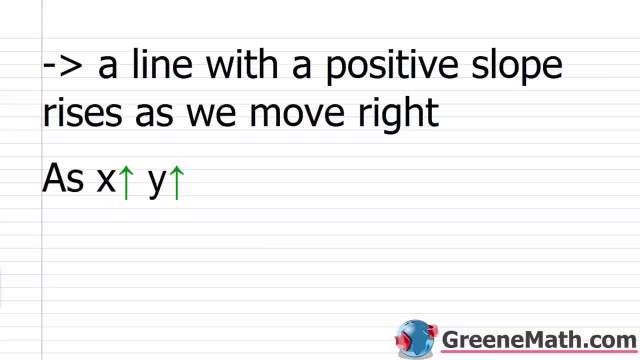 Alright so now that we have the basics down let's wrap up our lesson with a few basic things that you need to know about slope. 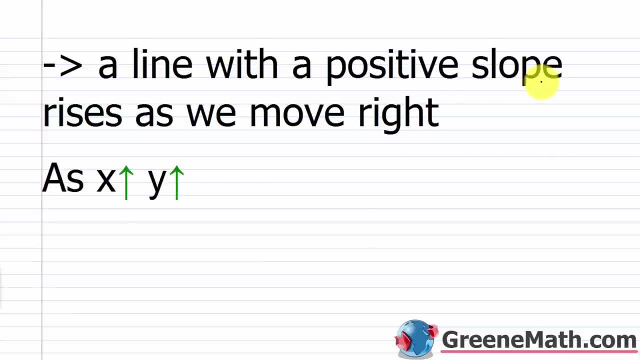 So the first thing is that a line with a positive slope rises as we move to the right. So that kind of looks like a line that does this. 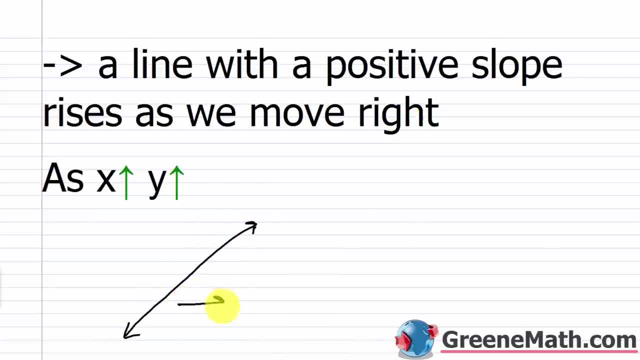 Alright so as we move to the right so as X increases. Remember X increases going to the right. Y increases. So as we go to the right the line is increasing in value. 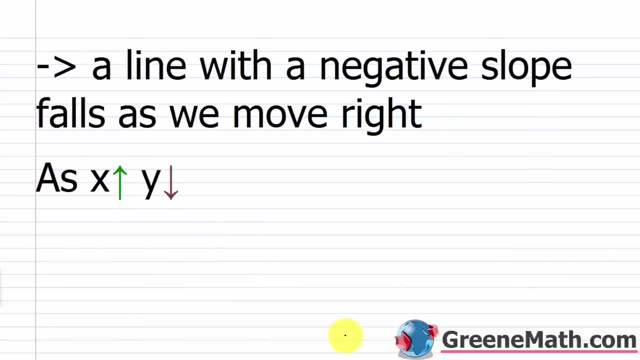 So similarly a line with a negative slope falls as we move to the right. 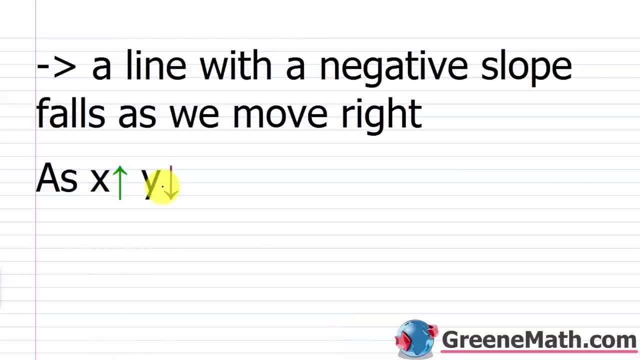 So in this case as X increases Y is now going to decrease. 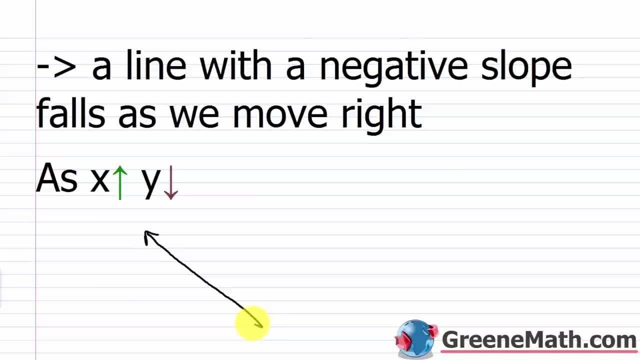 So that line would look something like this. 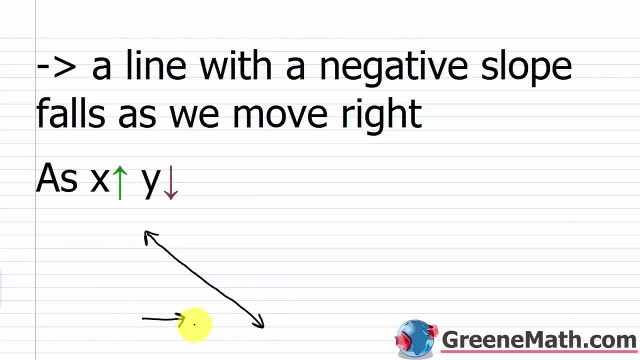 So as X is increasing remember X increases as we move to the right. 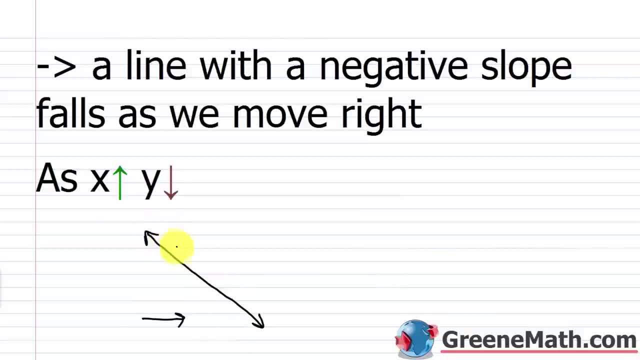 Y is now decreasing. Your vertical values are moving down as we go to the right. 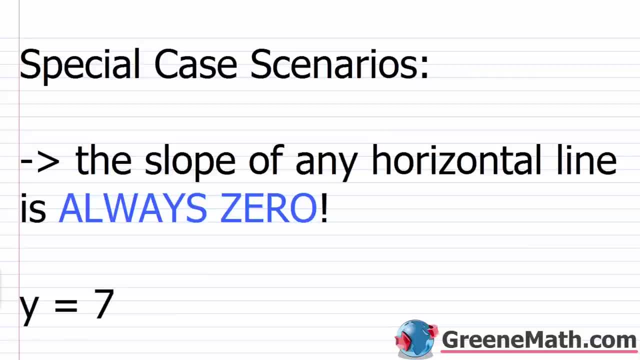 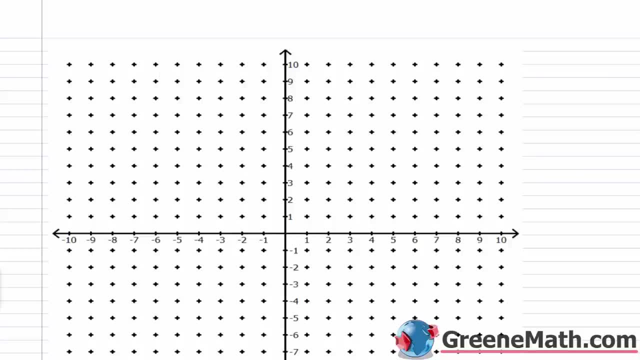 Alright let's talk about some special case scenarios. The slope of any horizontal line is always 0. So you have something like Y equals 7. So you'll recall graphically I just find 7 on the Y axis and I draw a horizontal line. That's how I graph that. 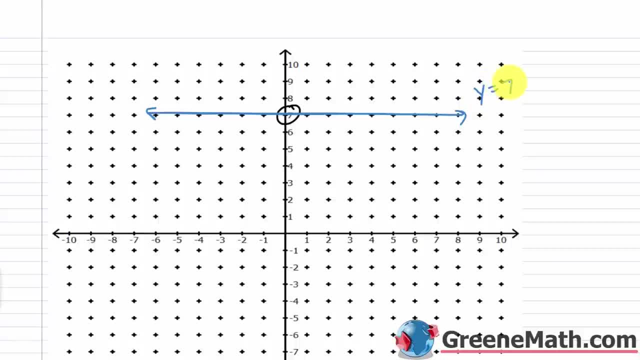 Okay so this could be my graph for Y equals 7. 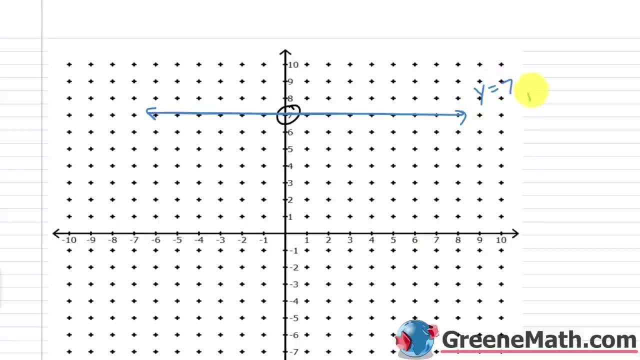 Now if we think about this in terms of again rise over run. So rise over run. 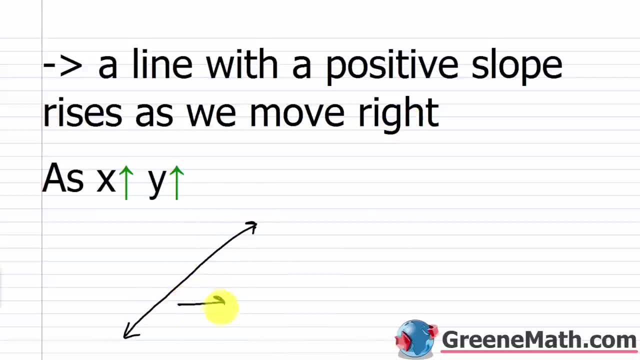 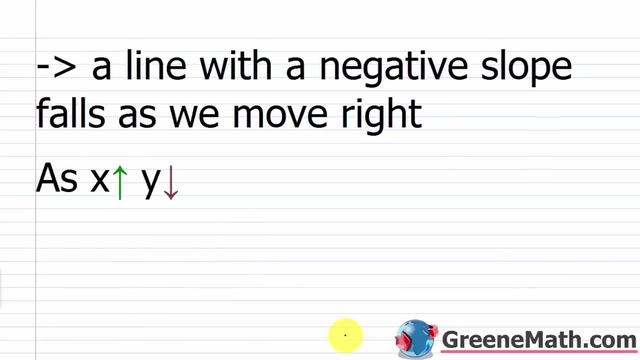 like a line that does this right. so as we move to the right, so as x increases- remember, x increases going to the right- y increases. so as we go to the right, the line is increasing in value. so, similarly, a line with a negative slope falls as we. 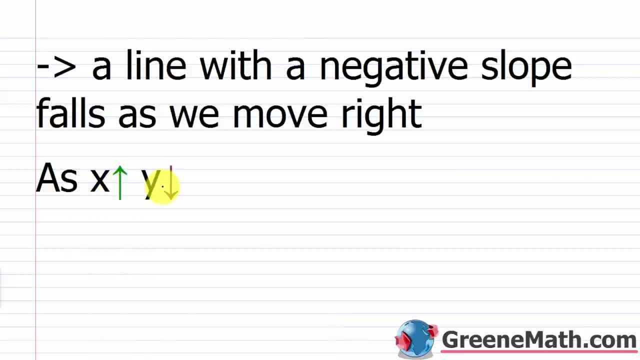 move to the right. as x increases, y is now going to decrease. so that line would look something like this: so as x is increasing- remember- x increases as we move to the right- y is now decreasing. your vertical values are moving down as we go to the right. 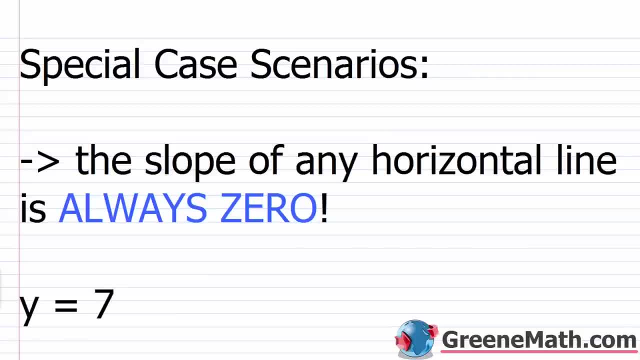 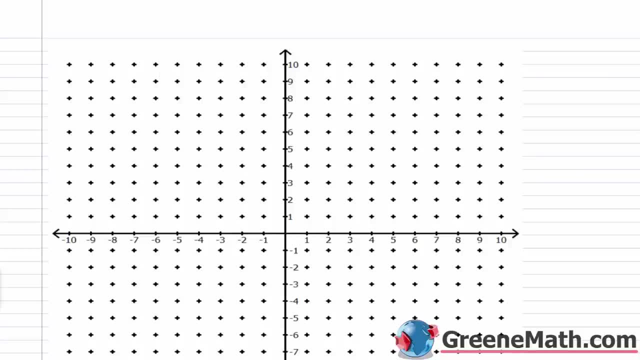 all right, let's talk about some special case scenarios. the slope of any horizontal line is always 0, so you have something like y equals 7, so you'll recall graphically, i just find 7 on the y-axis and I draw a horizontal line. that's how I graph that. okay, so this could be my. 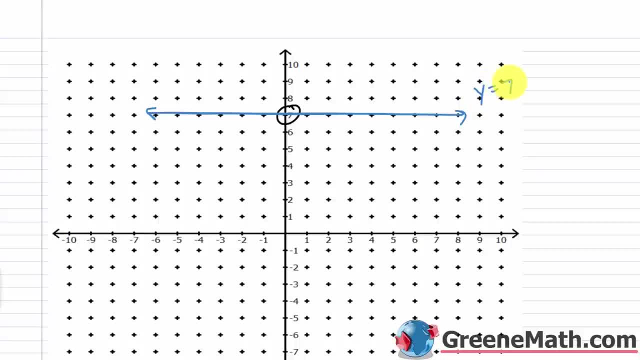 graph for y equals 7. now if we think about this in terms of again, rise over run, so rise over run, just think about moving one unit to the right. so let's say, I'm at this point right here and I go one unit to the right, so my run is 1. 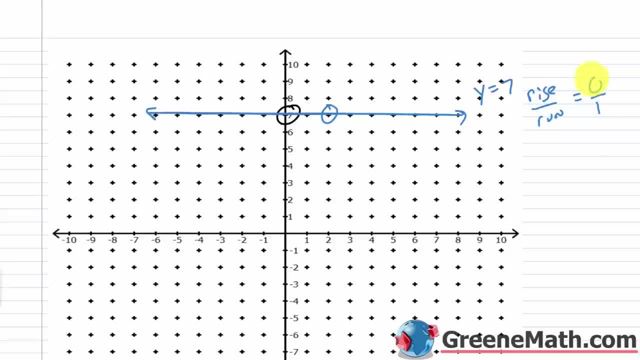 what's my rise? it's 0, and I'm not moving at all vertically, so I would have 0 over 1, which is just 0. right, take 0 and divided by any non 0 number, you get 0. so this is going to be the case every time we see a. 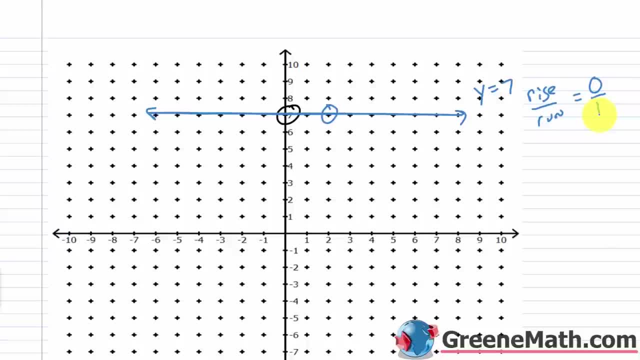 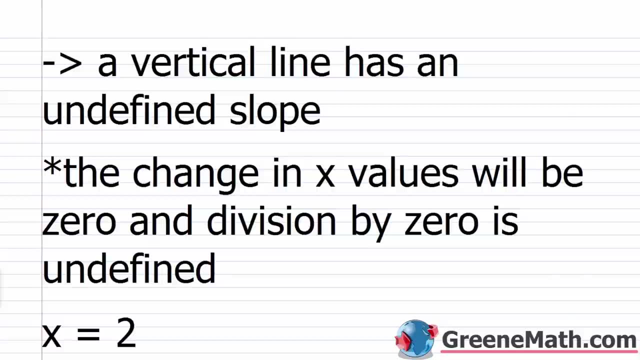 horizontal line. so a horizontal line has a slope that is 0. so, lastly, a vertical line has an undefined slope. this relates back to when I gave you the slope formula and I said x sub 2 could not equal x sub 1. well, again, you subtract. 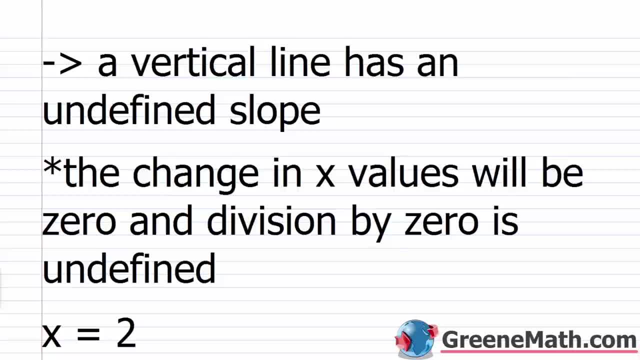 the same number from itself and you get 0. division by 0 is not allowed, so The change in x values will be 0, and division by 0 is undefined. So if I have a vertical line like x equals 2, you just say that the slope is undefined. 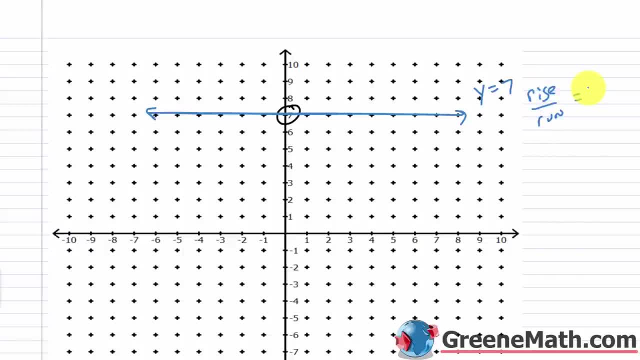 Just think about moving one unit to the right. So let's say I'm at this point right here and I go one unit to the right. So my run is 1. What's my rise? It's 0. 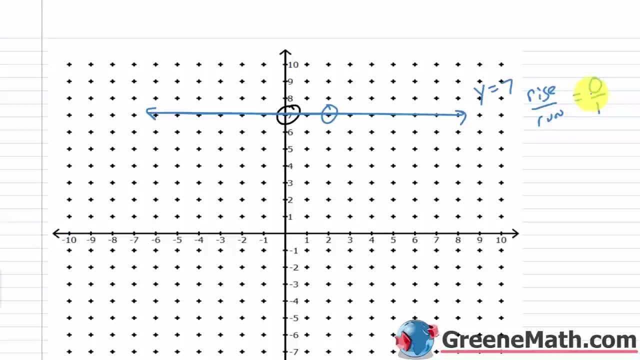 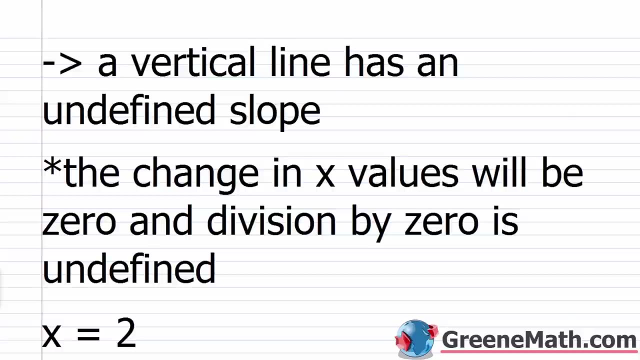 I'm not moving at all vertically. So I would have 0 over 1 which is just 0. Take 0 and divide it by any non-zero number and you get 0. So this is going to be the case every time we see a horizontal line. So a horizontal line has a slope that is 0. So lastly a vertical line has an undefined slope. 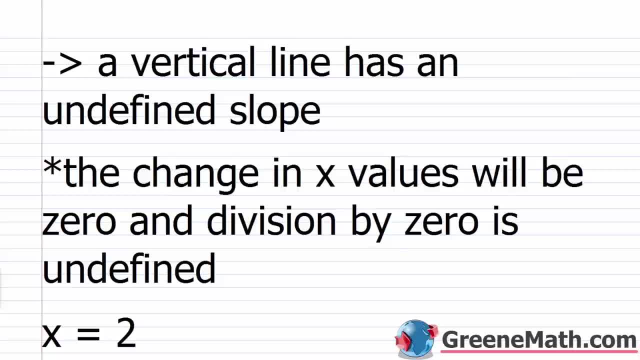 This relates back to when I gave you the slope formula and I said X sub 2 could not equal X sub 1. Well again you subtract the same number from itself and you get 0. Division by 0 is not allowed. So the change in X values will be 0 and division by 0 is undefined. So if I have a vertical line like X equals 2. You just say that the slope is undefined. 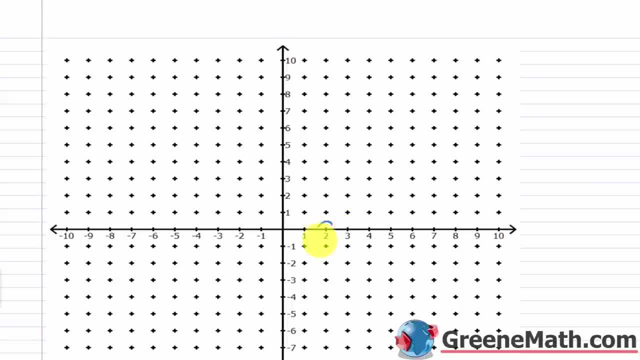 So if I saw X equals 2 on a graph remember I'd find 2 on the X axis. 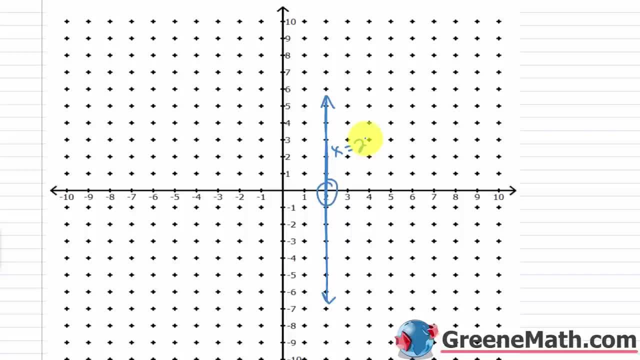 So again this is X equals 2. And if you think about this in terms of again rise over run. Just start it at any of these points and all of them are going to have the X location of 2. So let's say I start it out at this point. So this is 2 comma 3. 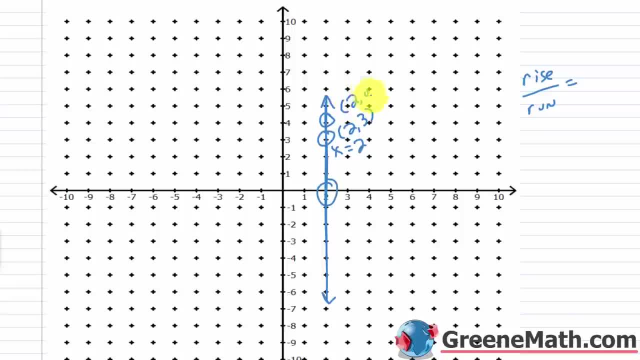 And I go to the next point above it which is 2 comma 4. Well my rise is 1 unit. Right? Because I increased on the Y axis by 1. But my run is 0. Right? My X location didn't change at all. So that's 0. And we're not allowed to divide by 0. 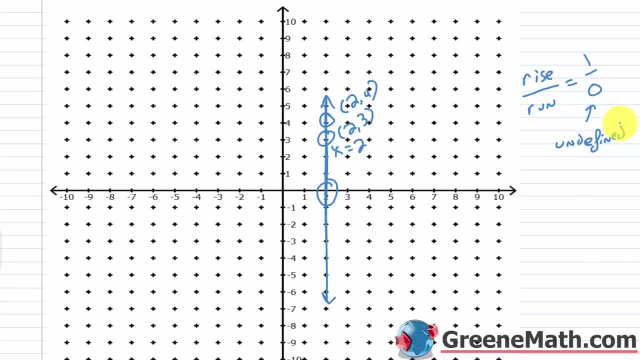 This is undefined. This is undefined. So when I have a vertical line and they ask you for the slope. You just reply that it's undefined. Because if you go to try to calculate it 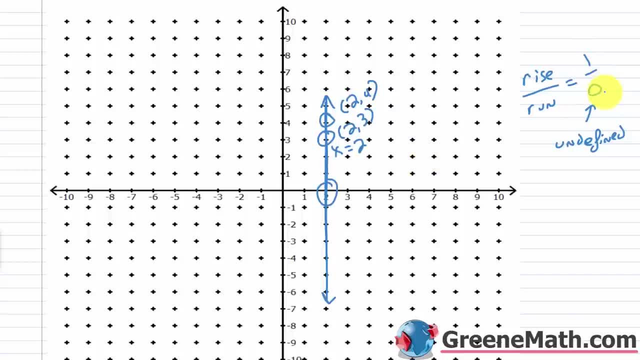 you're going to end up with division by 0. And once again that's 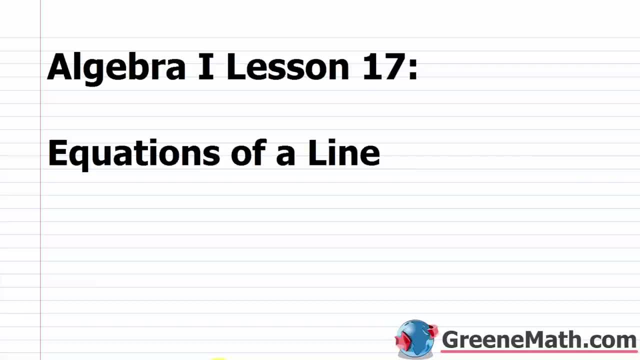 undefined. Hello and welcome to Algebra 1 lesson 17. 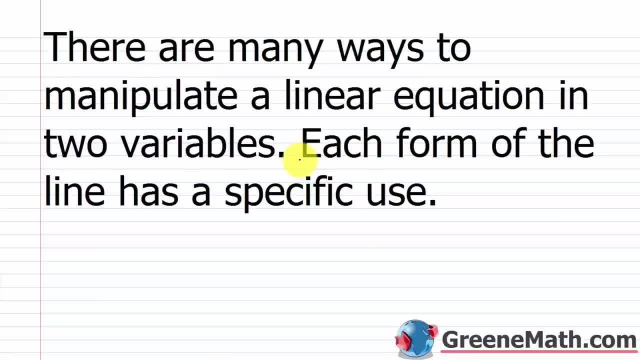 In this video we're going to learn about equations of a line. So as we continue in this chapter on linear equations in 2 variables. 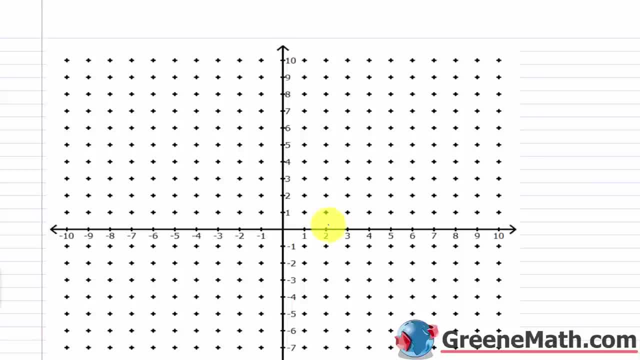 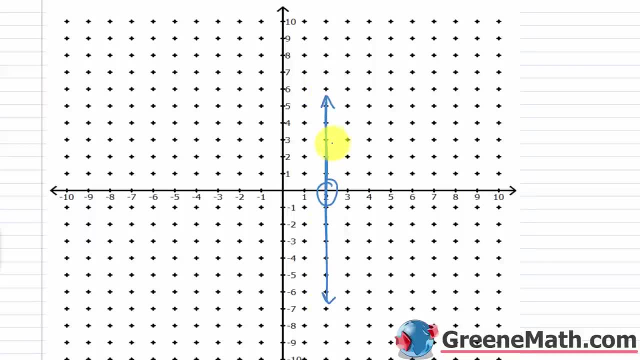 So if I saw x equals 2 on a graph, remember, I'd find 2 on the x-axis. So again, this is x equals 2.. And if you think about this in terms of again, rise over run, If you started at any of these points, and all of them are going to have the x location of 2.. 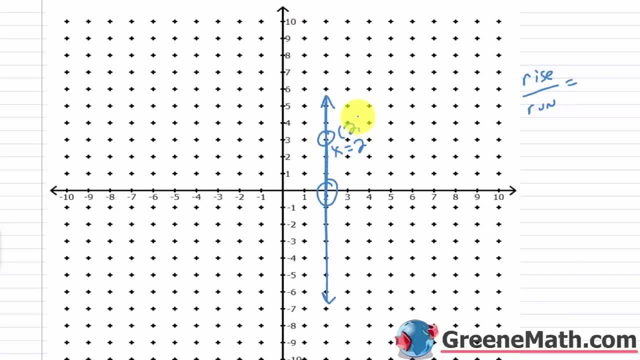 So let's say I started out at this point, So this is 2, 3.. And I go to the next point above it, which is 2, 4.. Well, my rise is 1 unit, right, Because I increased on the y-axis by 1.. 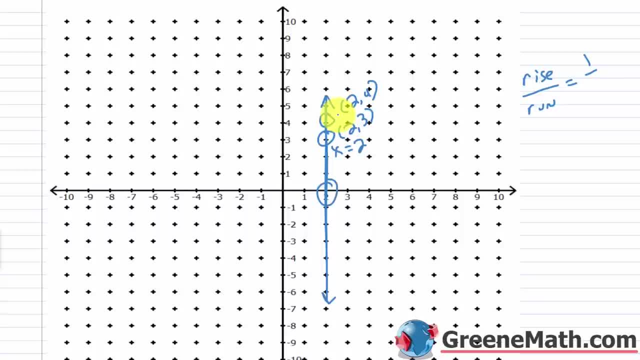 But my run is 0, right, My x location didn't change at all, So that's 0. And we're not allowed to divide by 0. This is undefined. This is undefined. So when I have a vertical line and they ask you for the slope, 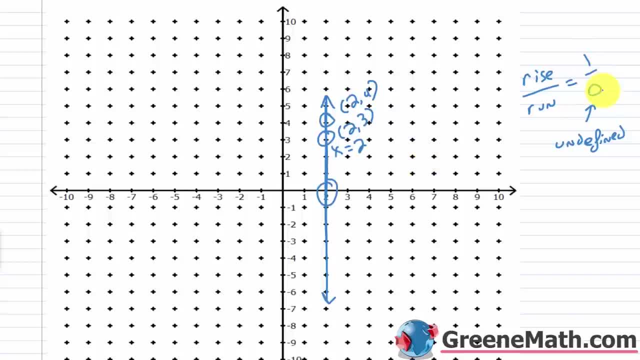 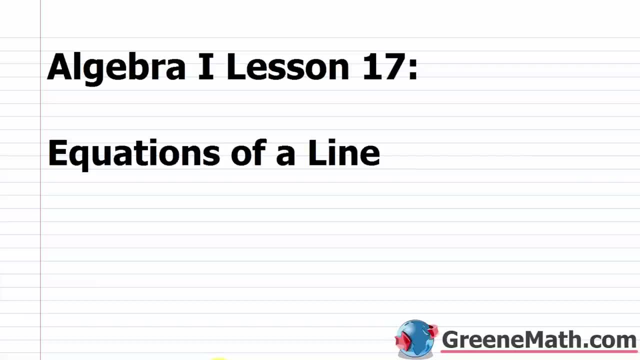 you just reply that it's undefined, Because if you go to try to calculate it, you're going to end up with division by 0. And once again, that's undefined. Hello and welcome to Algebra 1,, Lesson 17.. 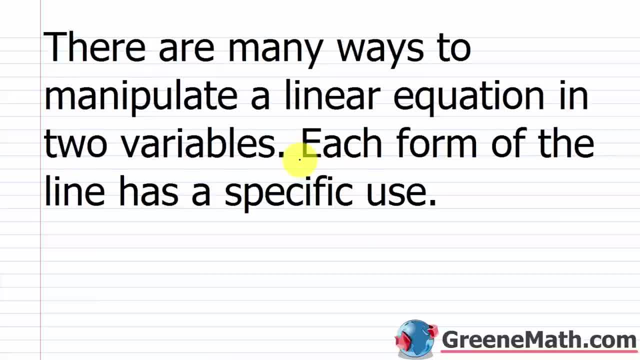 In this video we're going to learn about equations of a line. So, as we continue in this chapter on linear equations in two variables, we're going to now see that there are ways to manipulate a linear equation In two variables, and each form of the line has a specific use. 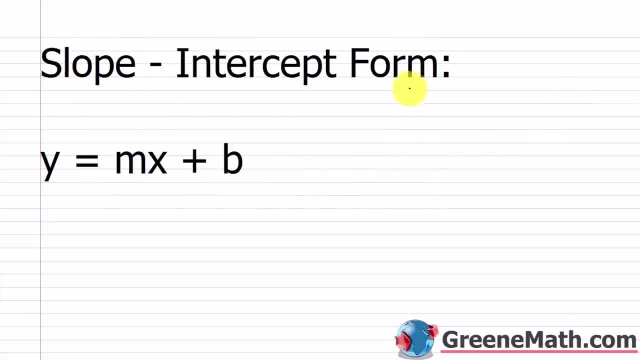 So kind of the most immediate would be slope intercept form, And this form of the line is very, very useful to us When we look at something in slope intercept form. we know the slope and the y intercept And that's why it's called slope intercept form. 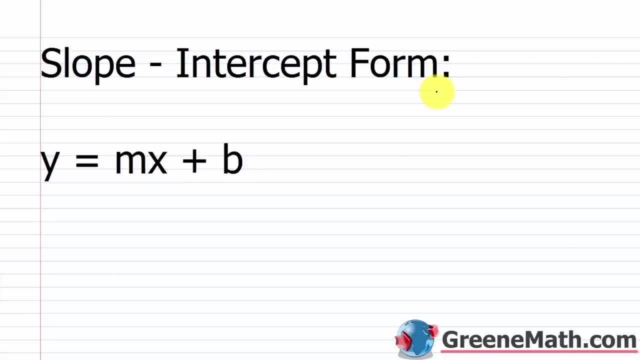 So if I have a linear equation in two variables and I solve it for y, meaning y is on one side of the equation by itself, like we have here- then we immediately know that m, the coefficient of x, is the slope. 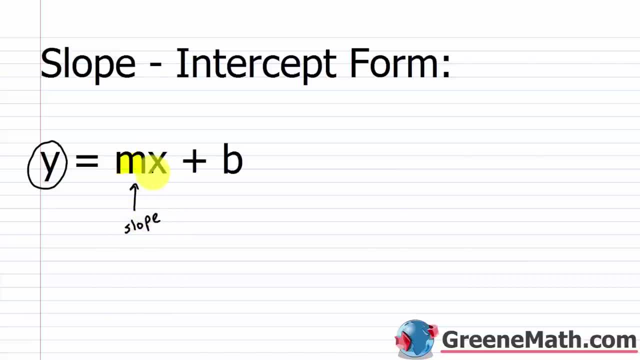 This is the slope, And you'll recall that in the last lesson, when I taught you the slope formula, I denoted slope using m. So it's no coincidence that we put m here next to x, because, again, m stands for slope. 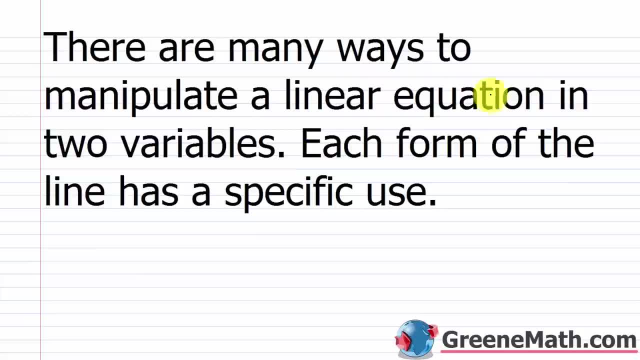 We're going to now see that there are ways to manipulate a linear equation in 2 variables. And each form of the line has a specific use. 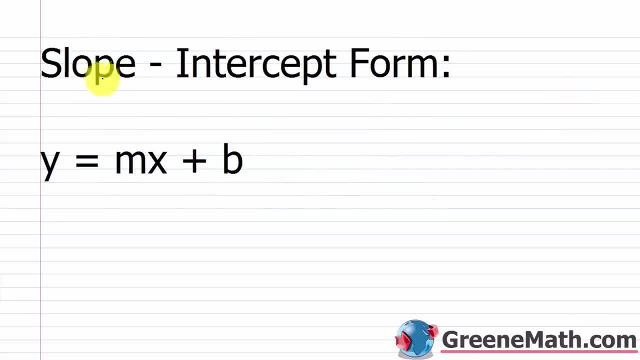 So kind of the most immediate would be slope intercept form. 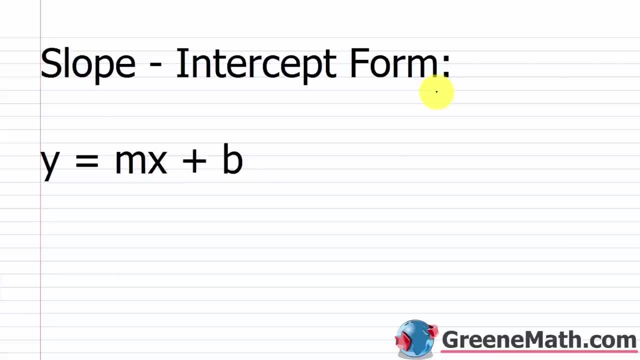 And this form of the line is very very useful to us. When we look at something in slope intercept form we know the slope and the y intercept. And that's why it's called slope intercept form. So if I have a linear equation in 2 variables and I solve it for y. Meaning y is on one side of the equation by itself like we have here. Then I immediately know that m the coefficient of x is the slope. 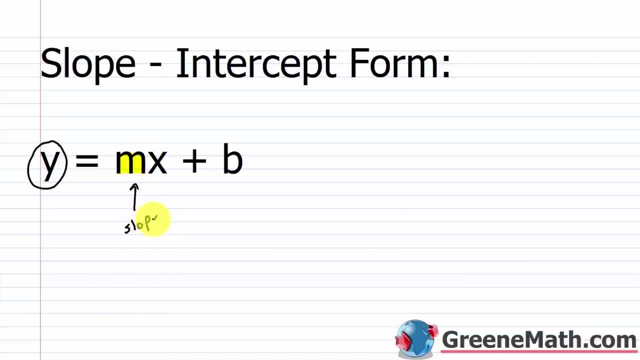 This is the slope. And you'll recall that in the last lesson when I taught you the slope formula I denoted slope using m. So it's no coincidence that we put m here next to x because again m stands for slope. Then plus b. Now this part right here is denoting our y intercept. 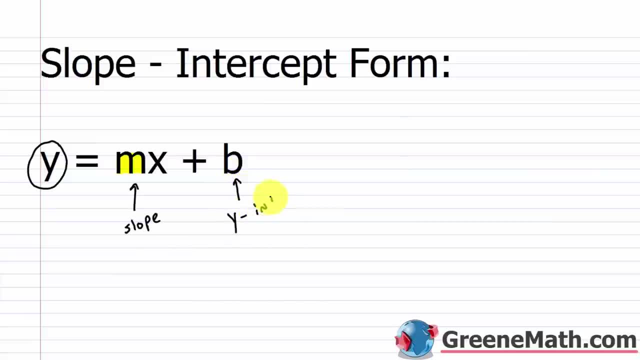 So this is your y intercept. And that's going to occur at 0 comma b. So whatever b is that's the coordinate for your y intercept. That's the y part of it. You'll have 0 always as the x coordinate when you're looking at your y intercept. And then b will be the y coordinate for your y intercept. 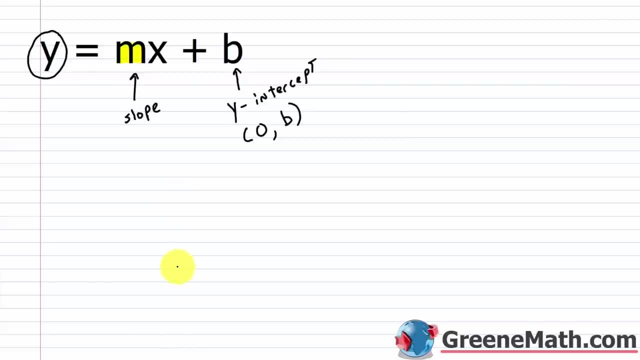 So as a quick example let me just give you a generic linear equation in 2 variables. Let's say I had something like 4x plus 2y equals negative 10. Really really simple. So if I want to get y by itself. If I want to solve it for y like I have up here. 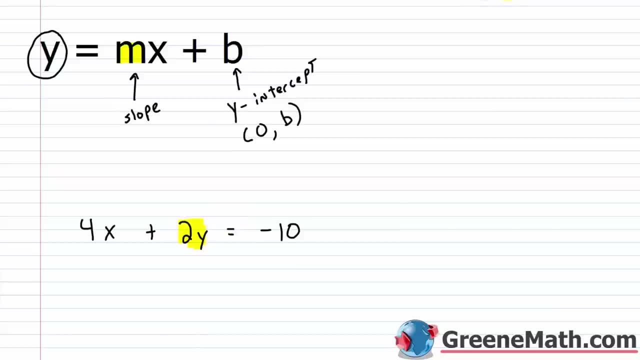 The first thing I need to do is just isolate this term 2y. So I would subtract 4x away from each side of the equation. And so this would go away. And on the left I'd have just 2y. 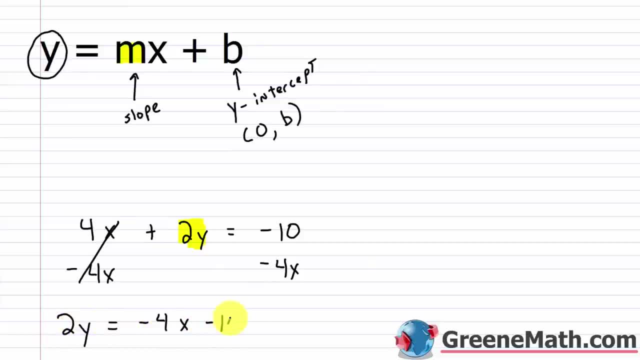 On the right I'd have negative 4x minus 10. 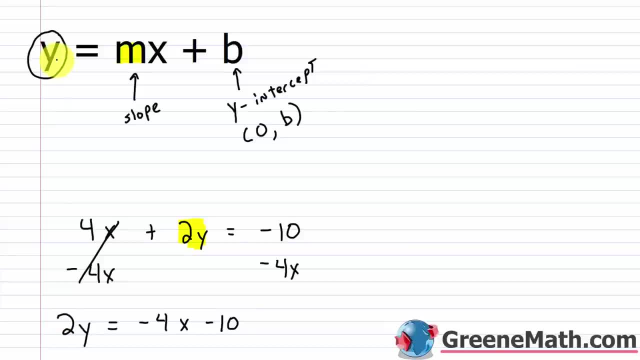 Now to isolate y to get it in this format I would just divide both sides of the equation by 2. 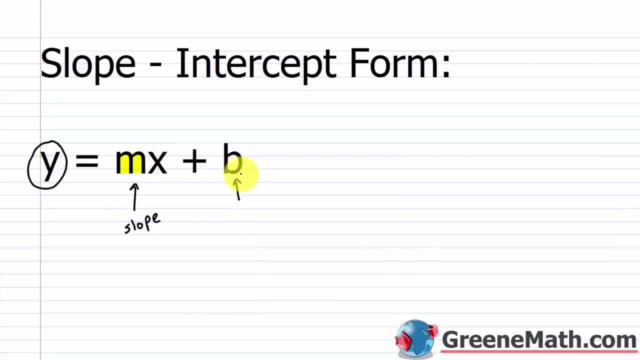 Then plus b. Now this part right here is denoting our y intercept. So this is your y intercept and that's going to occur at zero comma b. So whatever b is, that's the coordinate for your y intercept, right? 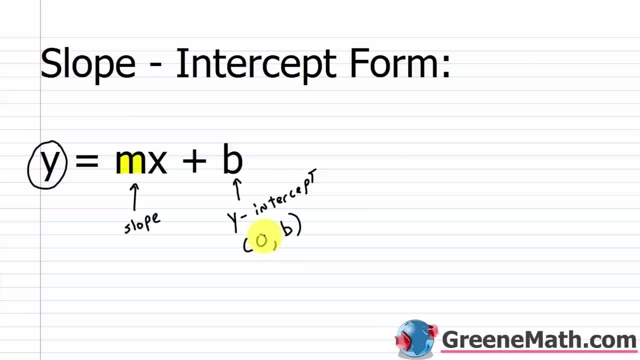 That's the y part of it. You'll have zero always as the x coordinate when you're looking at your y intercept, and then b will be the y coordinate for your y intercept. So as a quick example, let me just give you a generic linear equation in two variables. 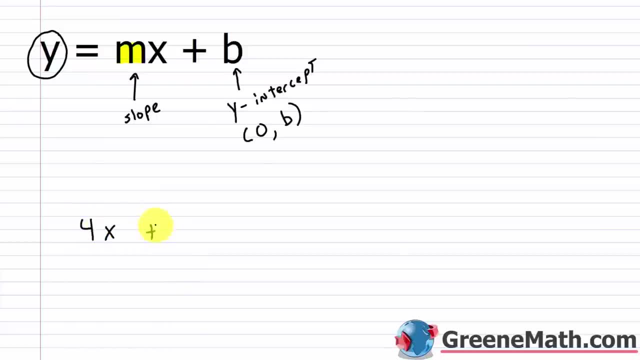 Let's say I had something like 4x plus 2y equals negative 10.. Really, really simple. So if I want to get y by itself, if I want to solve it for y like I have up here, the first thing I need to do is just isolate this term 2y. 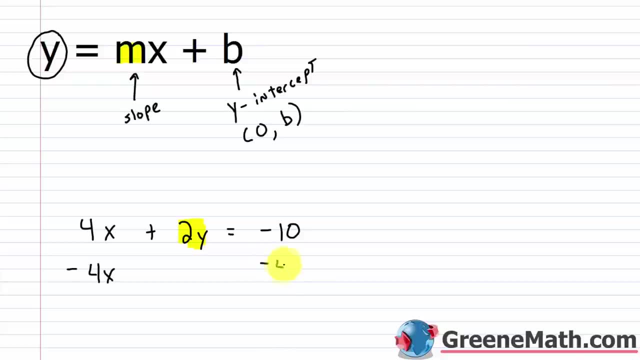 So I would subtract 4x away from each side of the equation And so this would go away, And on the left I'd have just 2y, On the right I'd have negative 4x minus 10.. Now to isolate y. 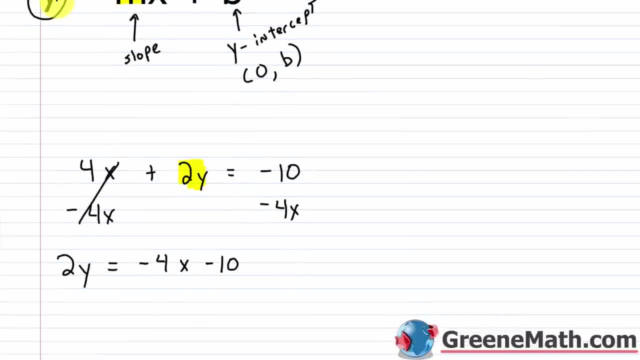 to get it in this format, I would just divide both sides of the equation by 2.. So I would divide this side by 2.. And a lot of students will just do this. They'll divide this by 2.. But remember, when you have a division like this: 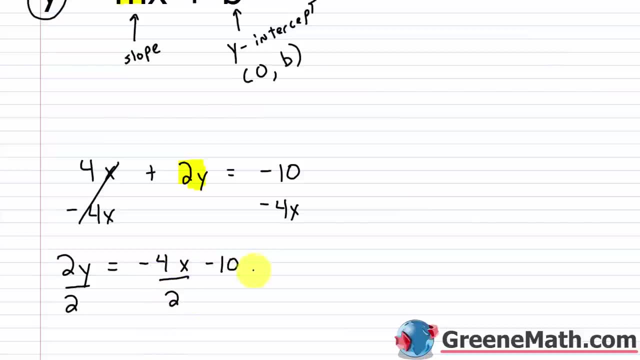 you're allowed to break it up and say: okay, I'm dividing this part by 2 and this part by 2.. Right, It's like having a common denominator, So you can do it that way. It makes it a little easier to simplify. 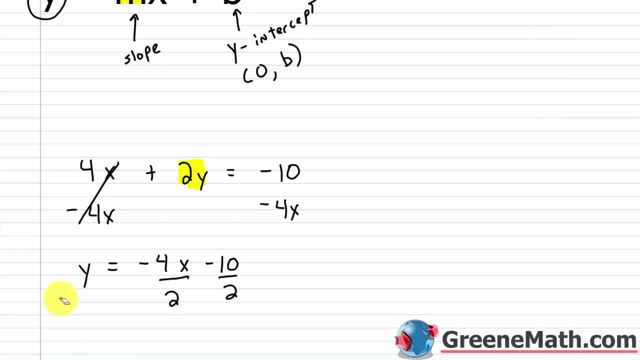 So this cancels with this and I'll just have y. And then negative 4 divided by 2 is negative 2.. So let's write that. Let's write that as negative 2.. And then negative 10 divided by 2 is negative 5.. 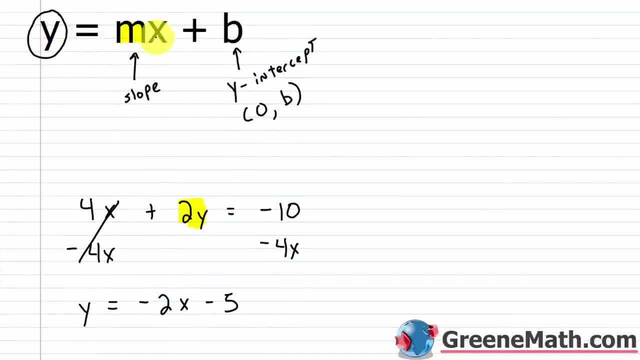 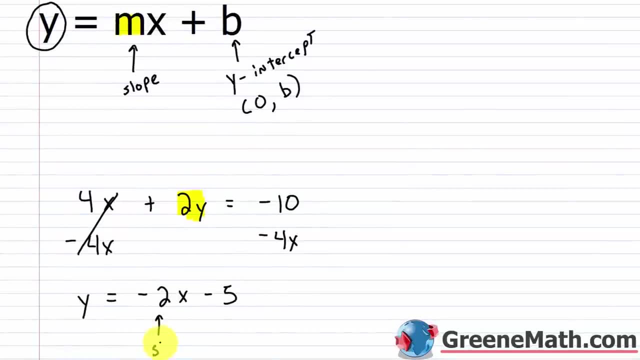 So, kind of looking up here, I have y equals m, the slope times x plus b, which is our y-intercept. So y equals negative 2x. So in this case negative 2 is the slope. This is your slope or your m. 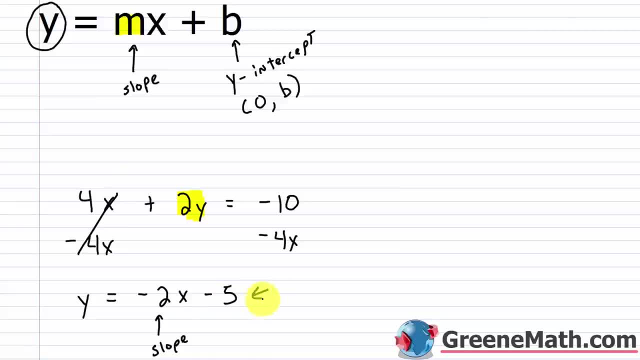 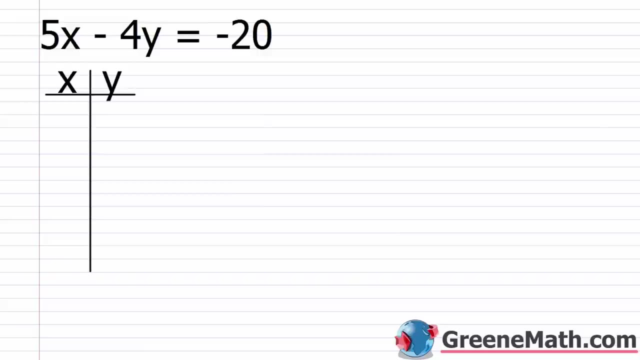 And then minus 5.. So minus 5, you can think of as plus negative 5.. So your y-intercept would occur at 0, comma negative 5.. This is your y-intercept, All right? so let's take a look at kind of an official example. 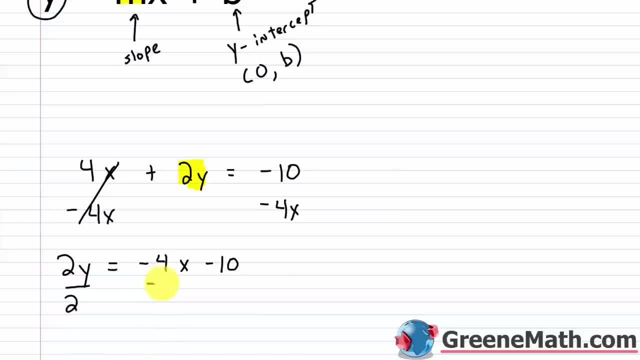 So I would divide this side by 2. And a lot of students will just do this. They'll divide this by 2. But remember when you have a division like this you're allowed to break it up and say okay I'm dividing this part by 2 and this part by 2. It's like having a common denominator. So you can do it that way. 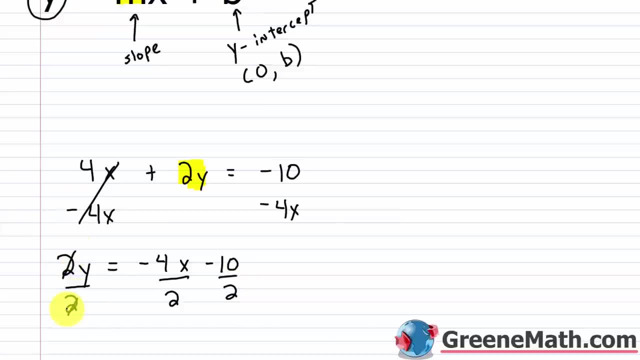 It makes it a little easier to simplify. So this cancels with this. And I'll just have y. And then negative 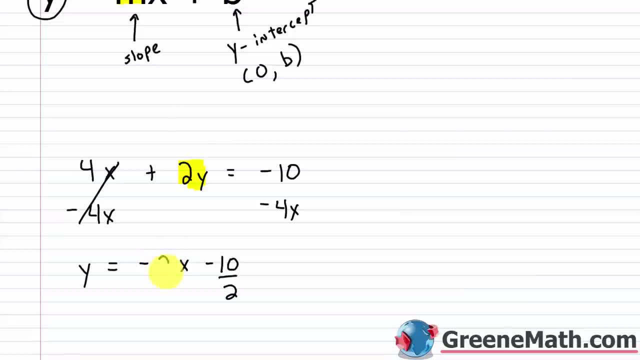 4 divided by 2 is negative 2. So let's write that as negative 2. 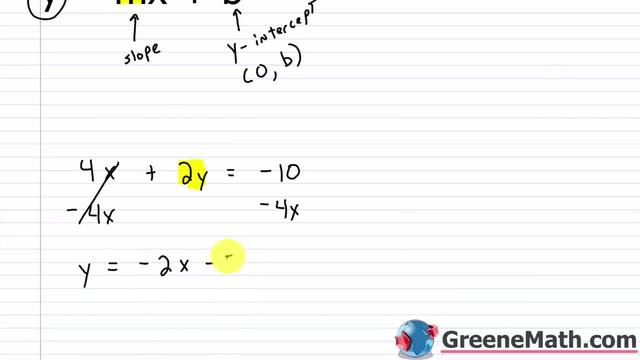 And then negative 10 divided by 2 is negative 5. 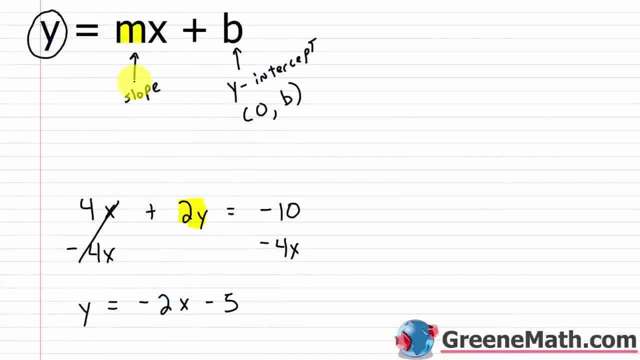 So kind of looking up here I have y equals m the slope times x plus b which is our y intercept. So y equals 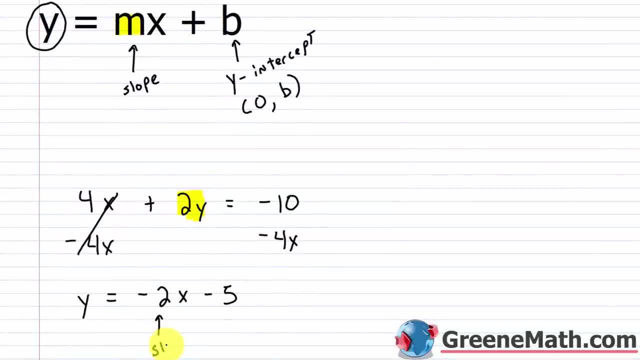 negative 2x. So in this case negative 2 is the slope. 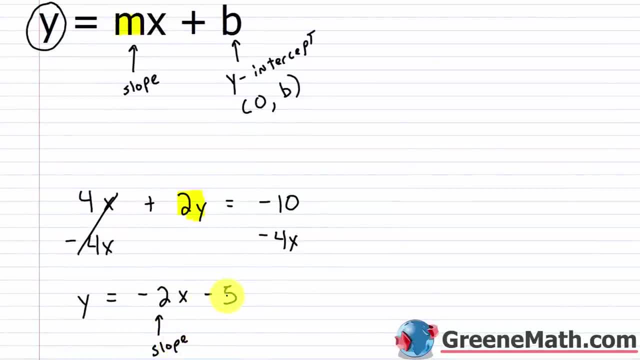 This is your slope or your m. And then minus 5. So minus 5 you can think of as plus negative 5. So your y intercept would occur at 0 comma negative 5. This is your y intercept. 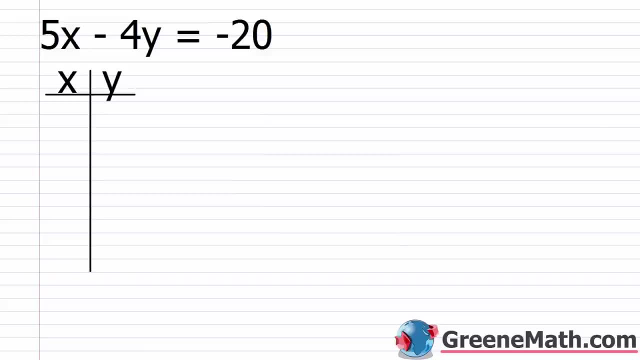 Alright so let's take a look at kind of an official example. And the reason for this example is I want to just convey to you in the past or kind of we'll just think about it in our last lesson we had to do a lot of work to find slope. You know if we're given an equation we had to calculate two points then go through and plug them into the slope formula and then now all we have to do is solve for y. Much much easier. But I'm going to show you the difference between kind of the old way and the new way. So we have our equation 5x 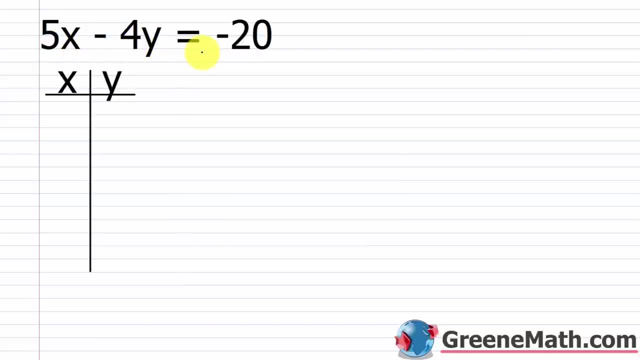 minus 4y equals negative 20. So old way I'd go through and get two points. So let's say I look for the y intercept. So that's me plugging in a 0 for x. So I'd have 5 times 0 minus 4y equals negative 20. So this would go away. And I'd have negative 4y equals negative 20. 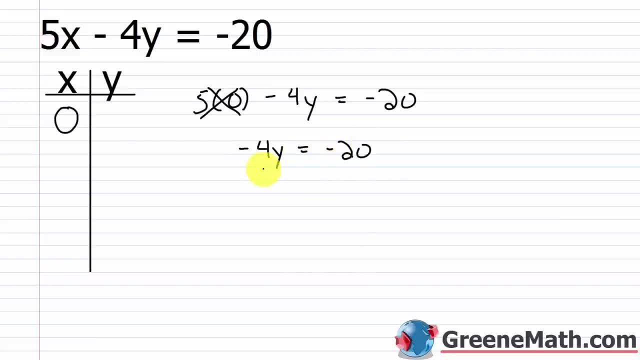 A lot of you can just look at that and say okay I know the answer is 5. But we'll officially say okay divide by negative 4 on each side. This cancels with this and you'll get y is equal to 5. 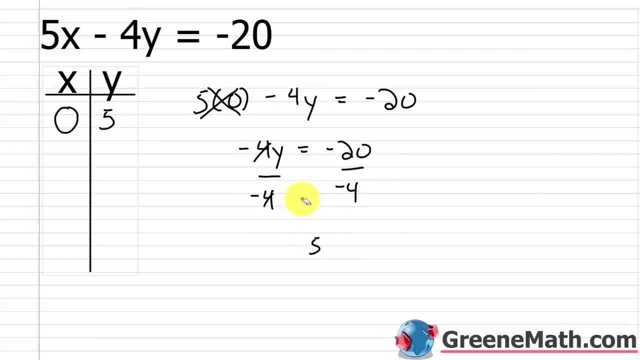 So if x is 0, y is 5. Okay. 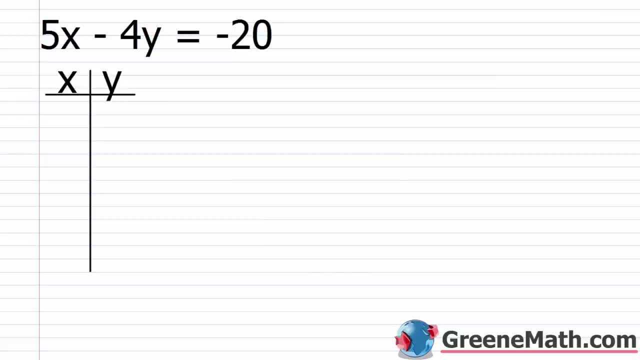 And the reason for this example is I want to just convey to you in the past, or kind of, we'll just think about it- in our last lesson we had to do a lot of work to find slope. You know, if we're given an equation, we had to calculate two points. 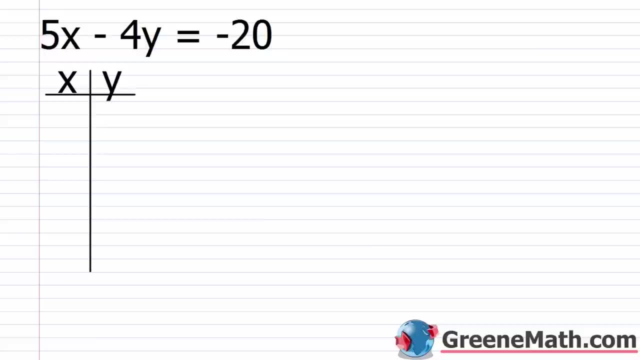 then go through and plug them into the slope formula and then now all we have to do is solve for y Much, much easier. But I'm going to show you the difference between kind of the old way and the new way. So we have our equation: 5x minus 4y equals negative 20.. 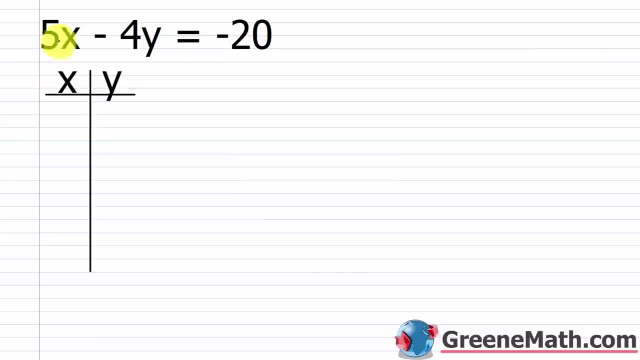 So old way I'd go through and get two points. So let's say I look for the y-intercept, So that's me plugging in a 0 for x. So I'd have 5 times 0 minus 4y equals negative 20.. 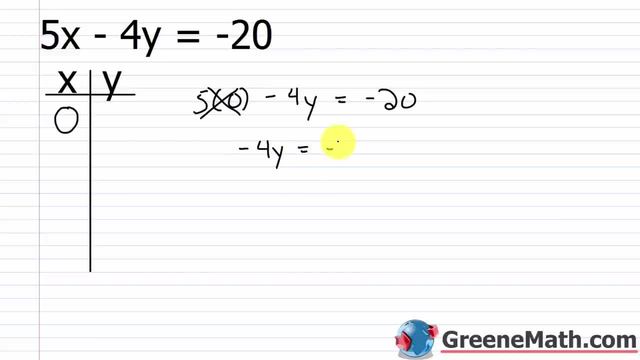 So this would go away and I'd have negative 4y equals negative 20.. A lot of you can just look at that and say, okay, I know the answer's 5.. But we'll officially say, okay, divide by negative 4 on each side. 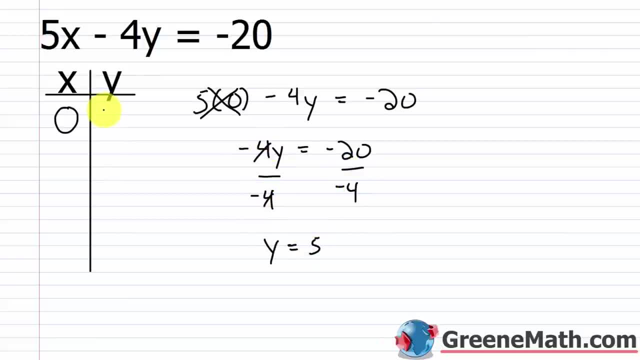 This cancels with this and you'll get: y is equal to 5.. So if x is 0,, y is 5.. Okay, Now let's go ahead and use the x-intercept. So that means y would be 0.. 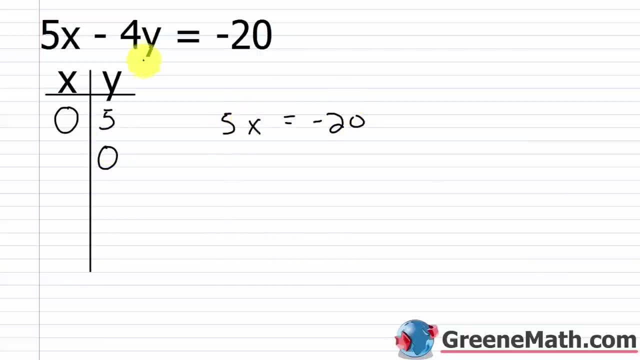 So I'd have: 5x is equal to negative 20, right, Because if I plug in a 0 there, negative 4 times 0 would just be 0. So that would just go away. So for this I would just solve by dividing both sides by 5.. 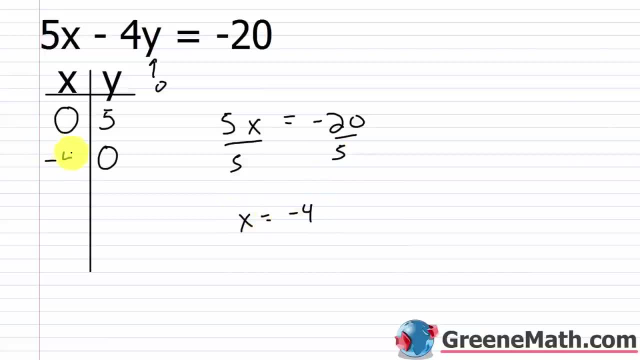 So then x would equal negative 4.. Okay, Very, very simple. So now I have two points. So one point is 0, 5.. And the other is negative 4, 0.. But now I need to plug these into the slope formula. 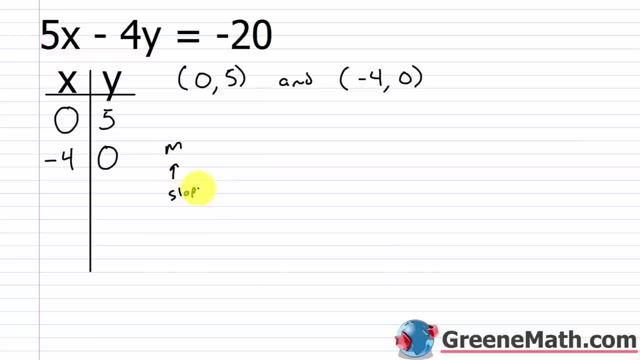 So remember m, which is the slope, is equal to y sub 2 minus y sub 1.. Over x sub 2 minus x sub 1.. All right, So let's label this one as x sub 1, y sub 1.. 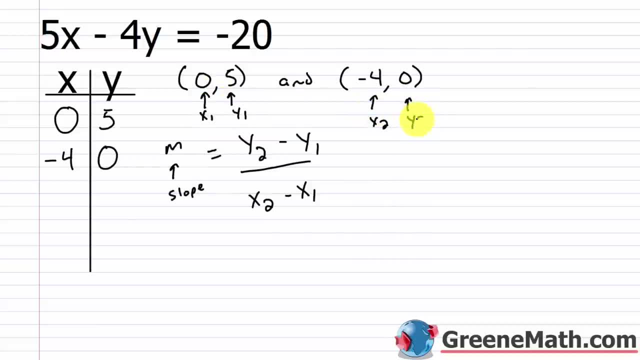 Let's label this one as x sub 2, y sub 2.. And let's see what happens when we plug in. So for y sub 2,, I have a 0.. So plug that in. For y sub 1, I have a 5.. 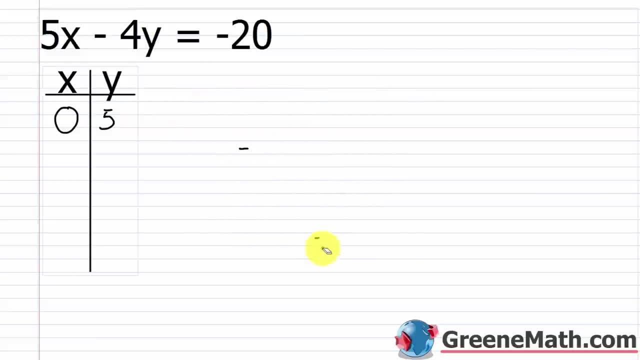 Now let's go ahead and use the x intercept. 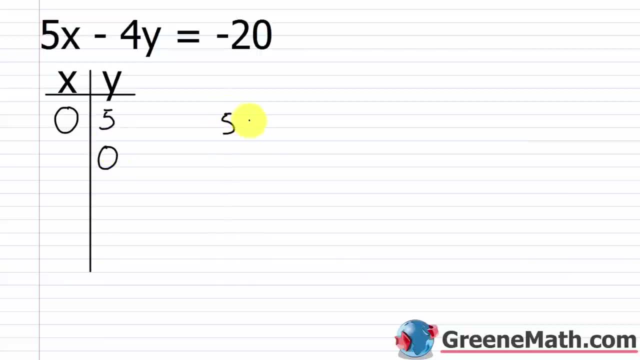 So that means y would be 0. So I'd have 5x is equal to negative 20. Right. Because if I plug in a 0 there negative 4 times 0 would just be 0. So that would just go away. So for this I would just solve by dividing both sides by 5. So then x would equal negative 4. Okay. 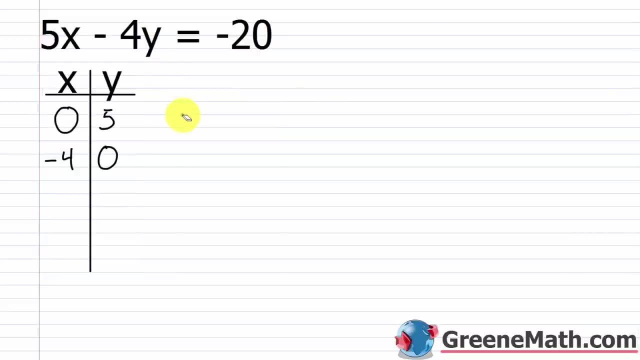 Very very simple. So now I have two points. So one point is 0 comma 5. And the other is negative 4 comma 0. But now I need to plug these into the slope formula. 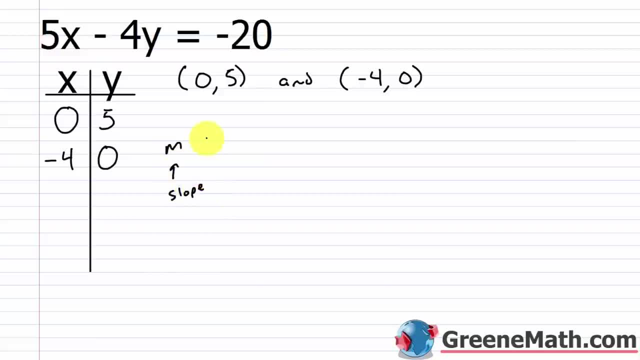 So remember m, which is the slope is equal to y sub 2 minus y sub 1 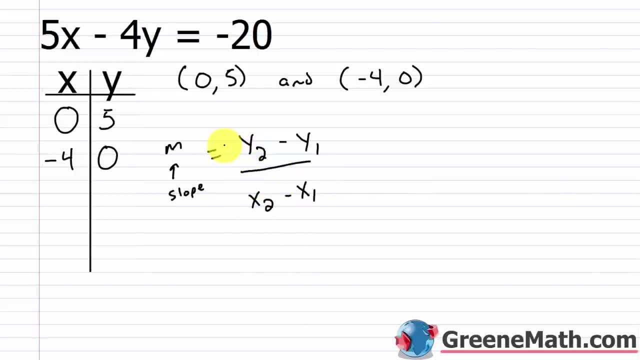 over x sub 2 minus x sub 1. Alright so let's label this one as x sub 1 y sub 1. Let's label this one as x sub 2 y sub 2. 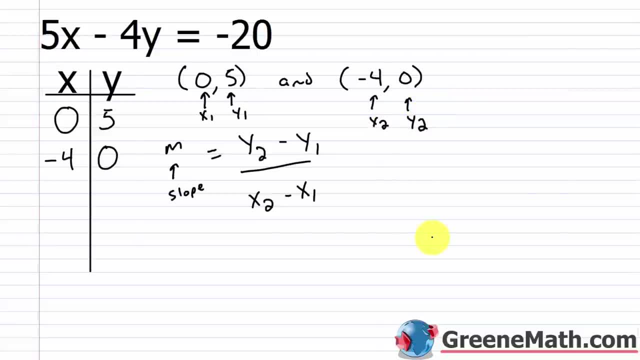 And let's see what happens when we plug in. So for y sub 2 I have a 0. So plug that in. For y sub 1 I have a 5. So plug that in. 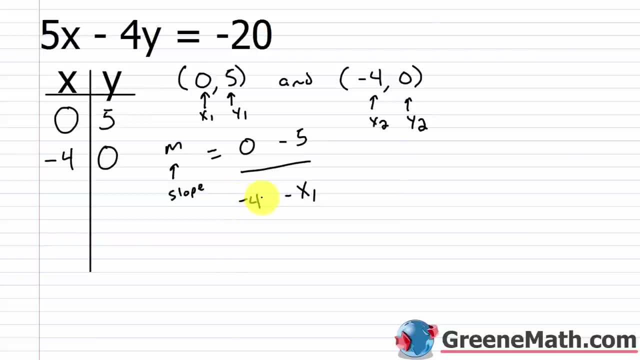 For x sub 2 I have a negative 4. Plug that in. And for x sub 1 I have a 0. 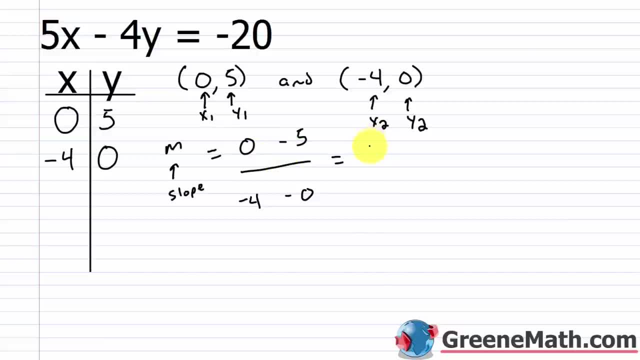 So plug that in. So 0 minus 5 is negative 5 over negative 4 minus 0 which is negative 4. So you get negative 5 over negative 4 which is 5 fourths. So that is your slope. And let's write that right here. That m equals 5 fourths. 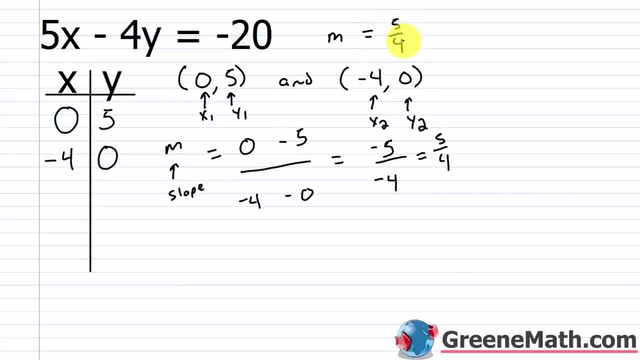 Now I'm going to show you something in two different ways. First off you saw how long and how complicated that process was just to figure out the slope. It's probably a minute, minute and a half, two minutes almost just to go through and get the first piece of information. Then you got to go back and plug it into the slope formula and get that. 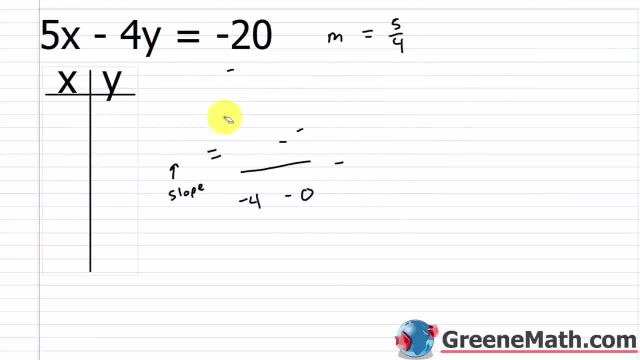 Let's erase this real quick. I'm going to show you a few different things. 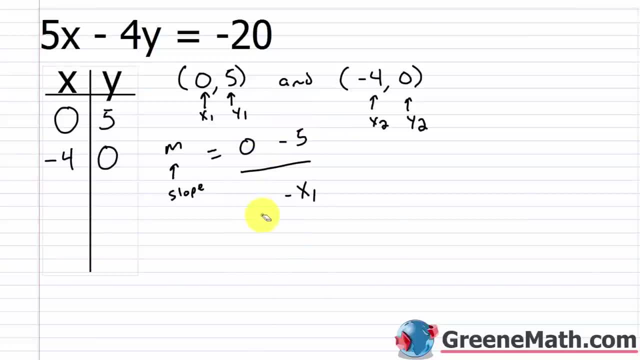 Plug that in. For x sub 2, I have a negative 4.. Plug that in. And for x sub 1, I have a 0. So plug that in. So 0 minus 5 is negative 5 over negative 4 minus 0, which is negative 4.. 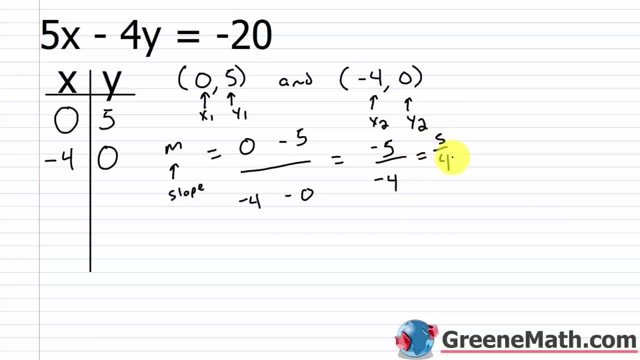 So you get negative 5 over negative 4,, which is 5 fourths. So that is your slope, And let's write that right here: That m equals 5 fourths. Now I'm going to show you something in two different ways. 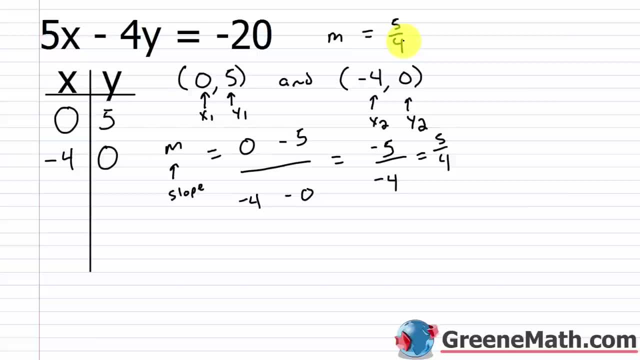 I mean, first off, you saw how long and how complicated that process was just to figure out the slope. I mean it's It's Probably a minute, minute and a half, two minutes almost, just to go through and get the first piece of information. 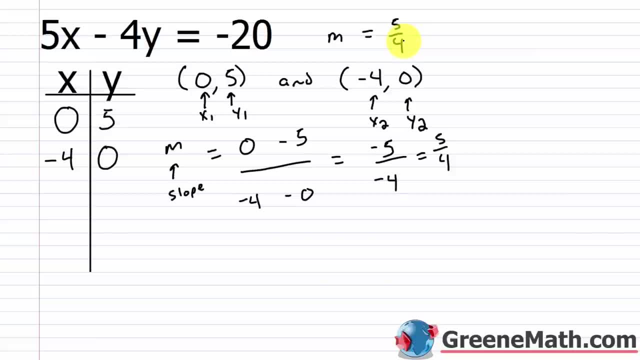 Then you got to go back and plug it into the slope formula and get that. So it's very, very time consuming. Let's erase this real quick. I'm going to show you a few different things. So the first thing I just want to show you- and this is kind of a side note- 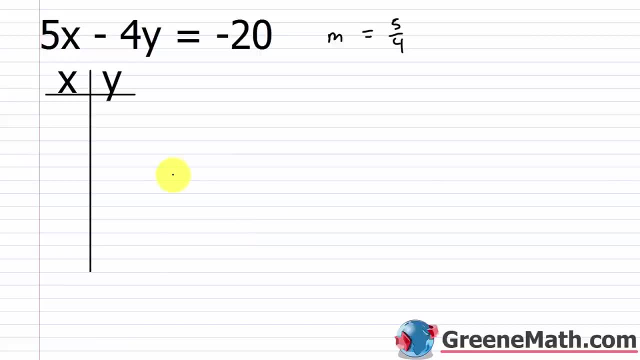 If you know the y-intercept which we figured that out it occurred at 0,5.. And you know the slope, You can write the equation in slope-intercept form. You have all the information you need. It's y equals m, the slope which is 5 fourths times x plus. 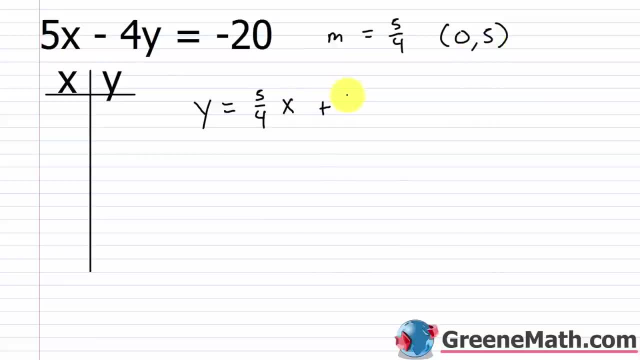 It's the y-coordinate from the y-intercept, So plus 5.. And you'll hear that they just say: this is the y-intercept, This is your y-intercept, And then this is the slope. Now I'm going to show you that I can take this equation right here and transform it into this one. 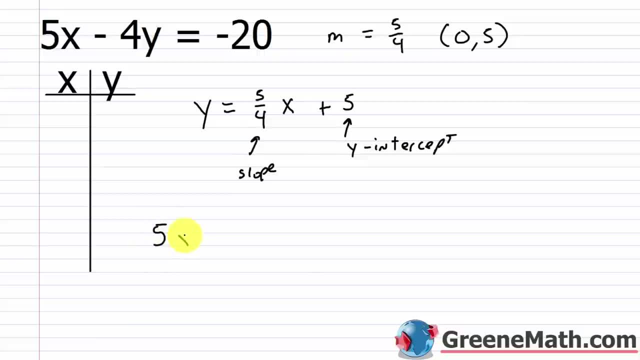 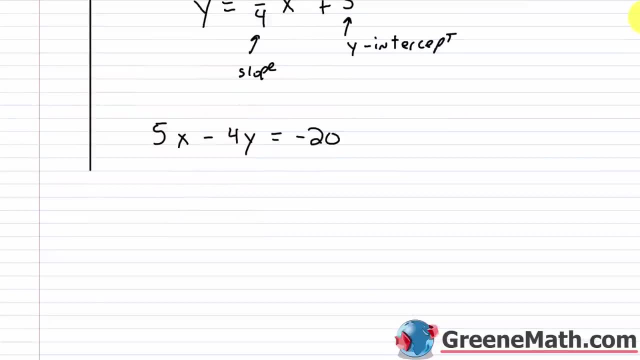 All I need to do is some basic algebra. So we have: 5x Minus 4y is equal to negative 20.. Let me scroll down a little bit just to get some room going. So again, if I want to isolate y, the first thing I need to do is isolate the negative 4y. 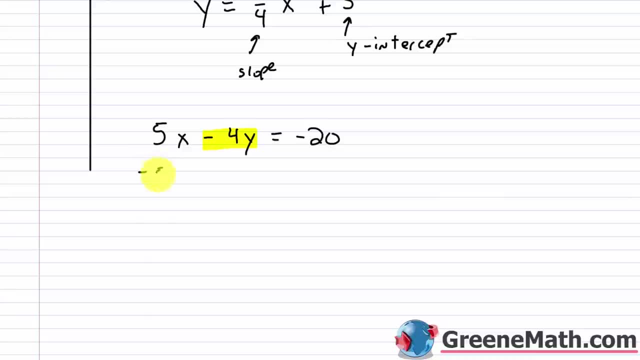 I'm going to isolate that whole term first, And to do that I would just subtract 5x away from both sides of the equation. Nice and simple. So that's gone. We'll have negative. 4y is equal to negative 5x minus 20.. 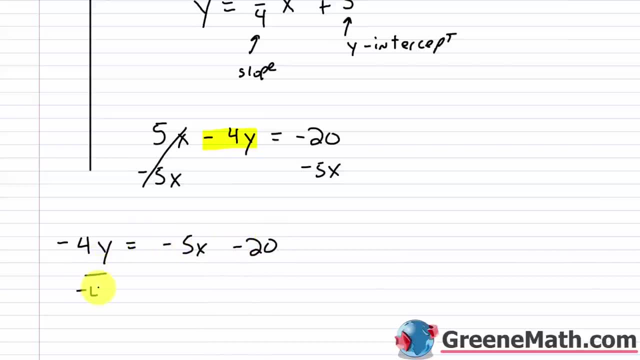 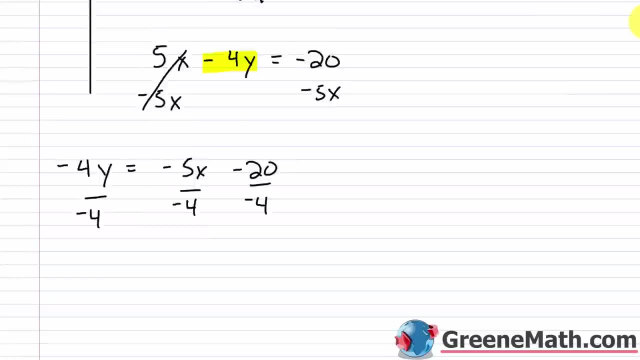 The next thing I want to do is get y by itself. So I'm going to divide by negative 4.. Divide over here by negative 4, and divide over here by negative 4.. So what are we going to have? Let's scroll down. 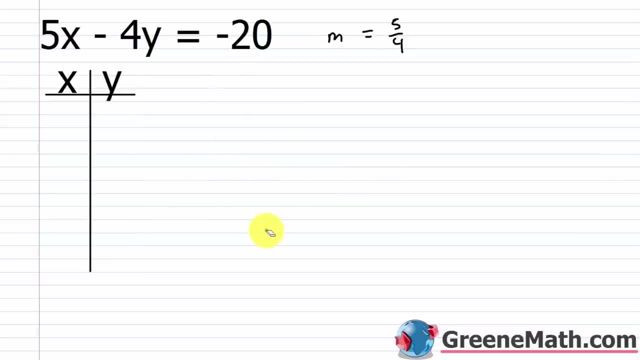 So the first thing I just want to show you and this is kind of a side note. If you know the y intercept which we figured that out it occurred at 0 comma 5 and you know the slope you can write the equation in slope intercept form. 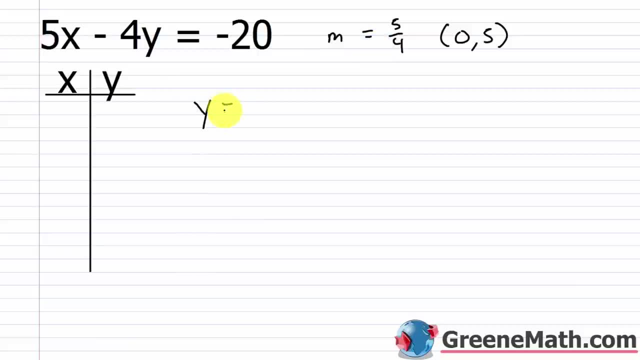 You have all the information you need. It's y equals m the slope which is 5 fourths times x plus it's the y coordinate from the y intercept. plus 5 and you'll hear that they just say this is the y intercept. This is your y intercept and then this is the slope. 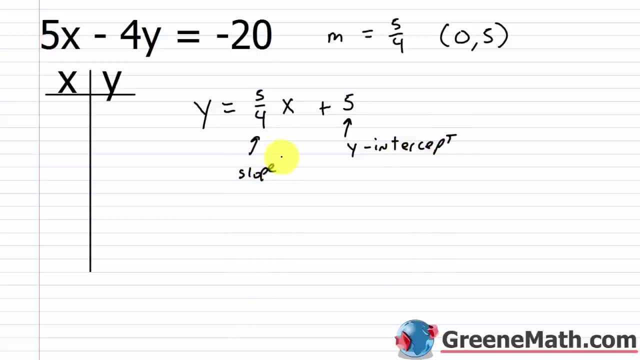 Now I'm going to show you that I can take this equation right here and transform it into this one. 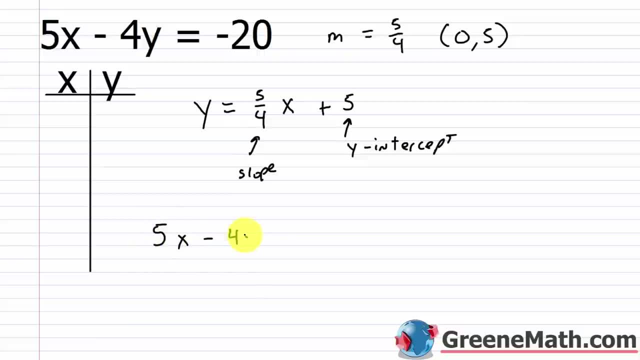 All I need to do is some basic algebra. So we have 5x minus 4y is equal to negative 20. 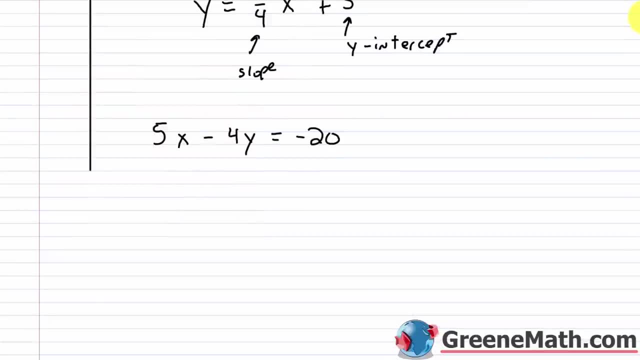 Let me scroll down a little bit just to get some room going. 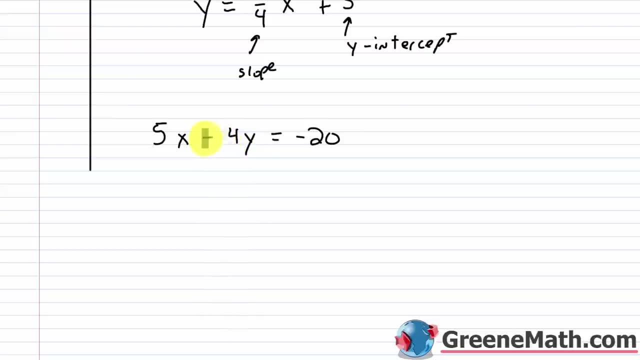 So again if I want to isolate y the first thing I need to do is isolate the negative 4y. I need to isolate that whole term first. And to do that I would just subtract 5x away from both sides of the equation. 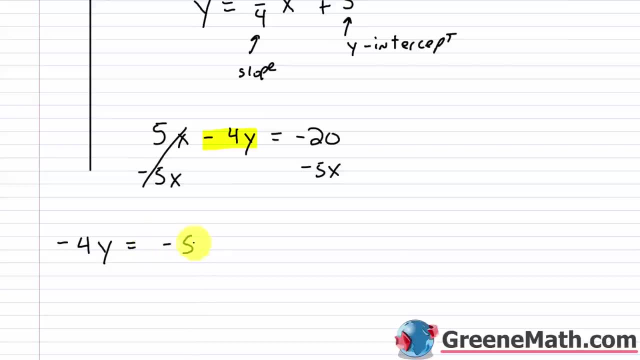 Nice and simple. So that's gone. We'll have negative 4y is equal to negative 5x minus 20. 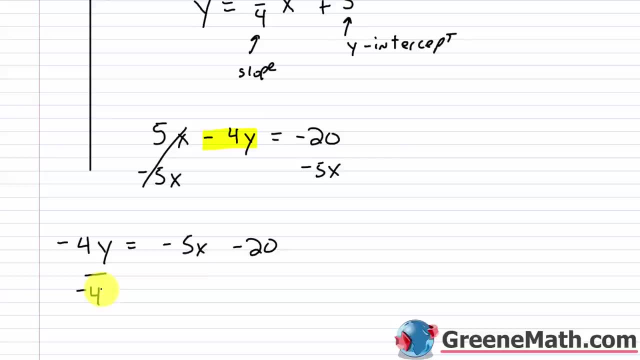 The next thing I want to do is get y by itself. So I'm going to divide by negative 4 divide over here by negative 4 and divide over here by negative 4. So what are we going to have? 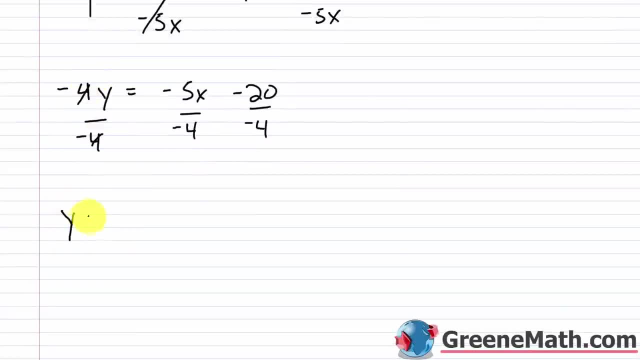 Let's scroll down. This will cancel with this 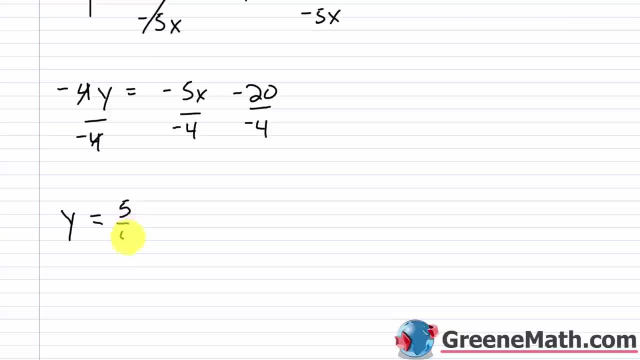 and I'll have y is equal to positive so that's 5 fourths then times x. 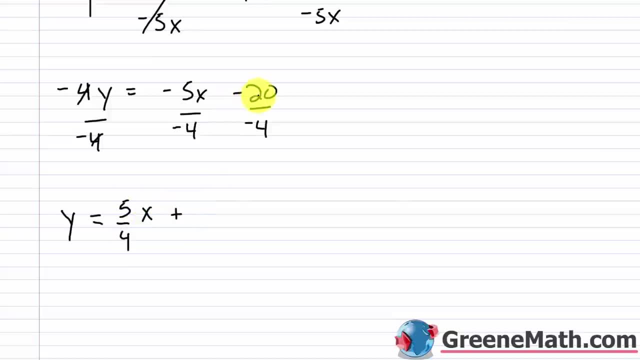 And then you can think of this as plus negative 20 so let's put a plus here. Negative 20 over negative 4 is 5. 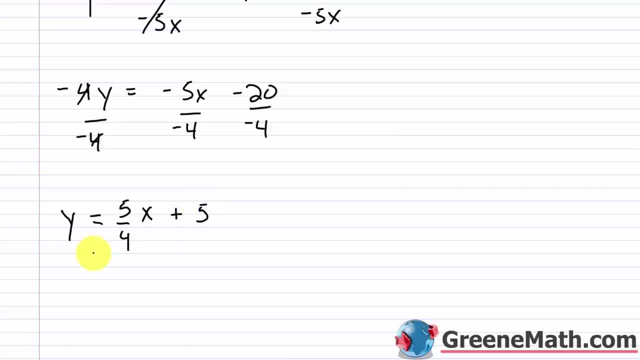 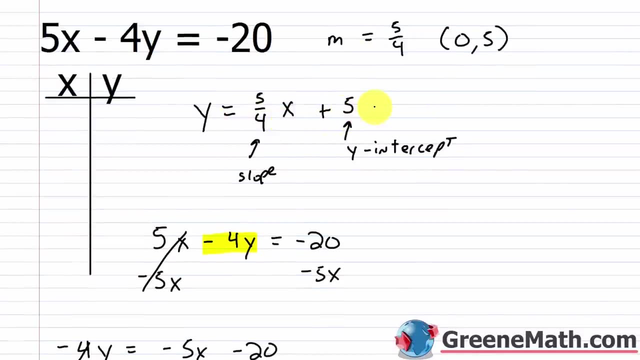 So what did we end up with? We end up with y equals 5 fourths x plus 5. And that is exactly what we had up here. Just by the given information. y equals 5 fourths x plus 5. 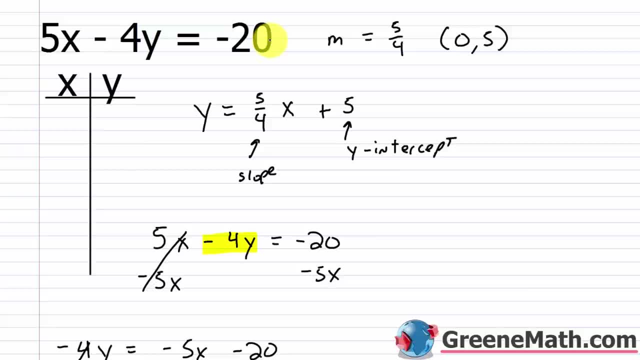 So if you have a linear equation in two variables you can solve it for y and you can immediately figure out the slope and the y intercept without going through getting points and then plugging it into the slope formula and so on and so forth. 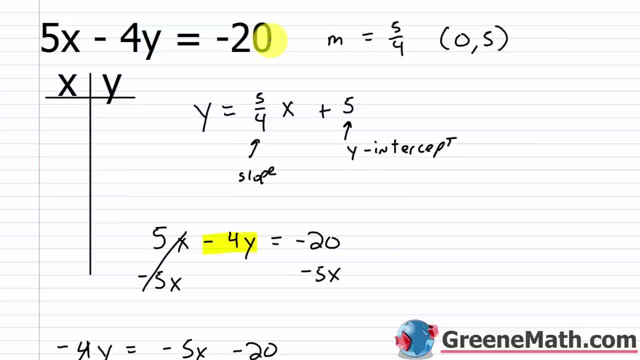 The other thing is if you're given the y intercept and you're given the slope you can just write the equation. 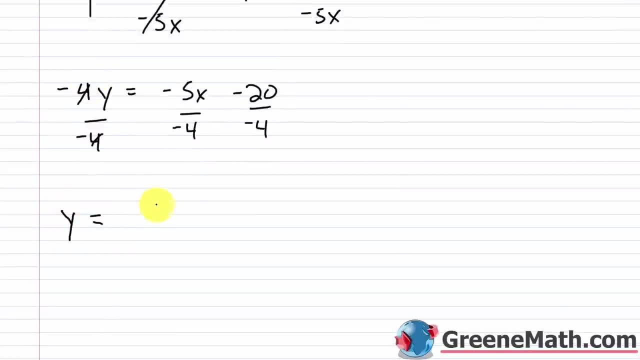 This will cancel with this and I'll have: y is equal to negative over negative is positive. so that's 5, fourths, then times x, And then you can think of this as plus negative 20, so let's put a plus here. 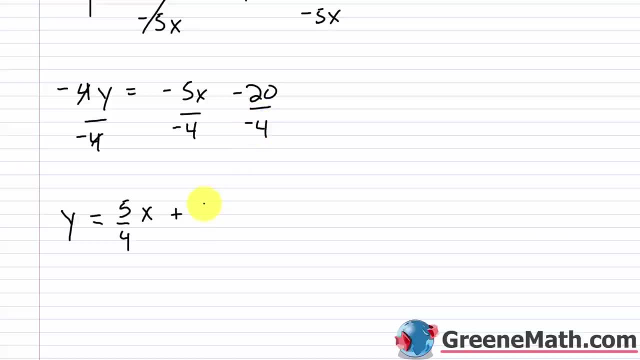 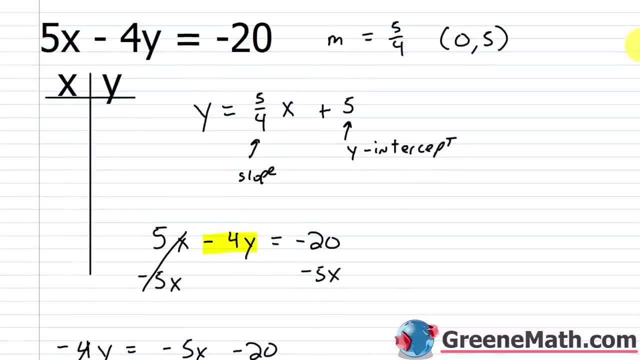 Negative 20 over negative 4 is 5.. So what did we end up with? We end up with: y equals 5 fourths x plus 5.. And that is exactly what we had up here, just by the given information, right. 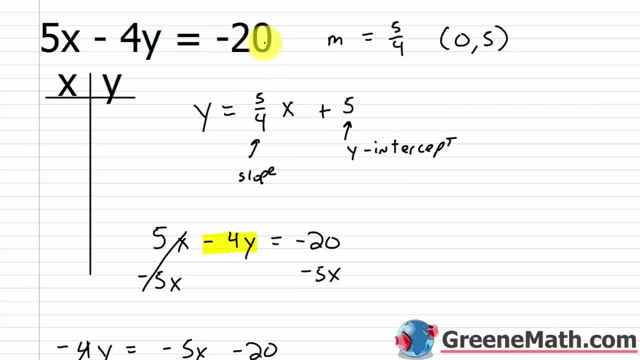 y equals 5 fourths x plus 5.. So if you have a linear equation in two variables, you can solve it for y and you can immediately figure out the slope and the y intercept without going through getting points and then plugging it into the slope formula and you know. so on and so forth. 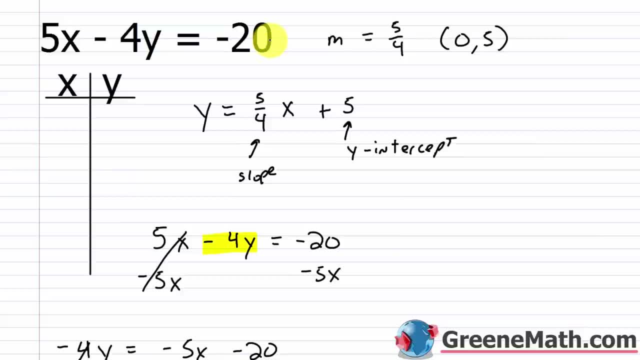 The other thing is, if you're given the y intercept and you're given the slope, you can just write the equation right Again. we're going to do that here in a little while, All right, so here's another example. 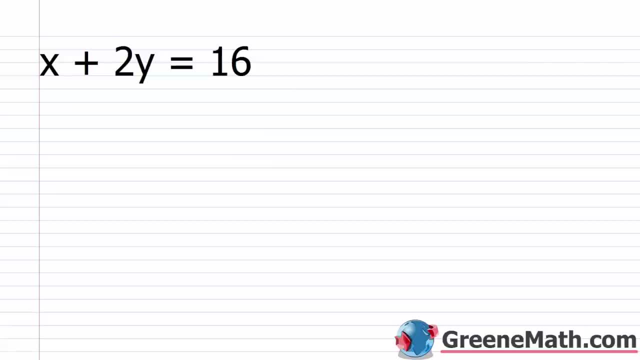 We have x plus 2y equals 16. And we don't need to go through any tedious process here. We're just going to solve this for y and we're going to figure out what our slope is, and we're also going to know what our y intercept will be. 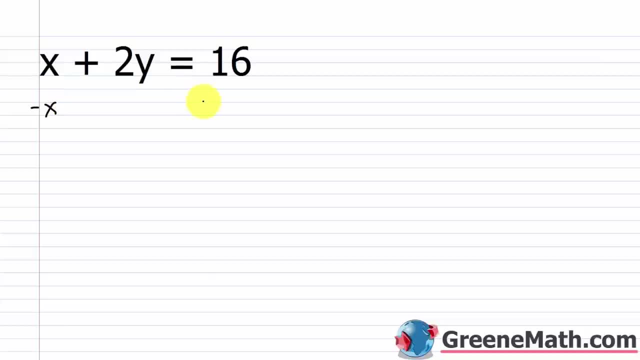 So to solve for y, I would subtract x away from each side, right, because I want to isolate this guy right here. So I would have: 2y is equal to negative x plus 16, and then I would divide each side of the equation by 2.. 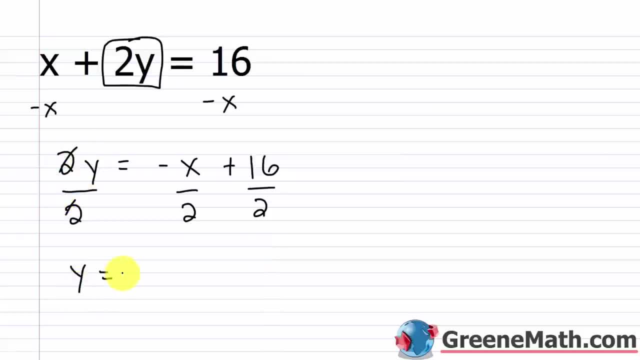 So what would I have? That would cancel. I'd have y is equal to You. think about negative x as negative 1 times x, right? We don't typically write that, but to make it clear, you have negative 1 half times x there. 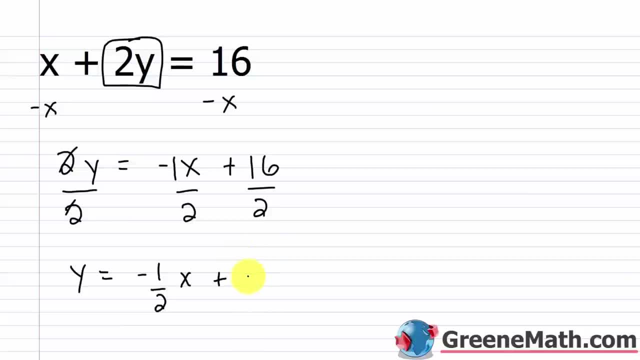 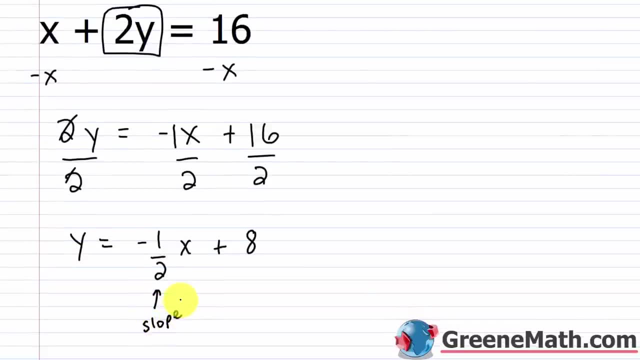 So negative 1 half times x plus 16 over 2 is 8.. So I have my equation solved for y, and now I know that the slope, or m, is negative 1 half and I know that the y intercept will occur at 0, 8.. 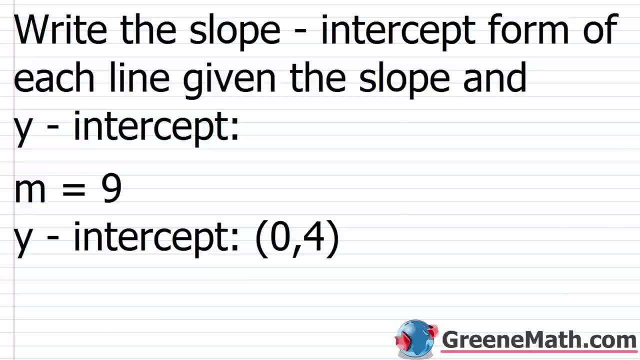 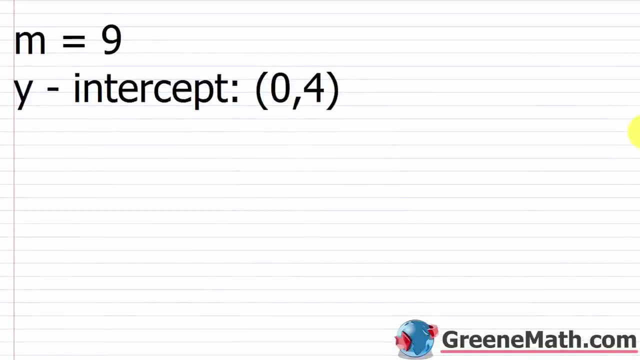 So here's another very common textbook-type example, something you'll probably get on your test. so we want to write the slope intercept form of each line, given the slope and y-intercept, and we just did this a little while ago. so we have that M equals 9 and again M is standing for. 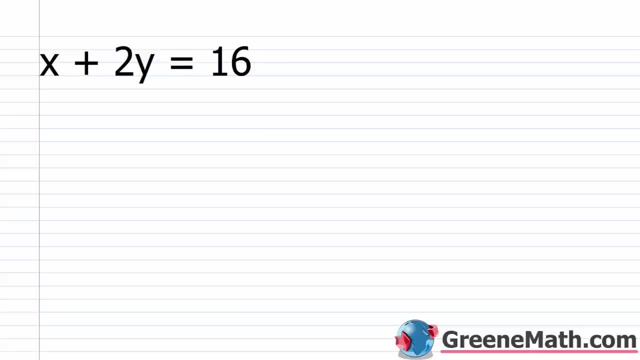 Again we're going to do that here in a little while. So here's another example. We have x plus 2y equals 16 and we don't need to go through any tedious process here. We're just going to solve this for y and we're going to figure out what our slope is and we're also going to know what our y intercept will be. So to solve for y we're going to subtract x away from each side because I want to isolate this guy right here. 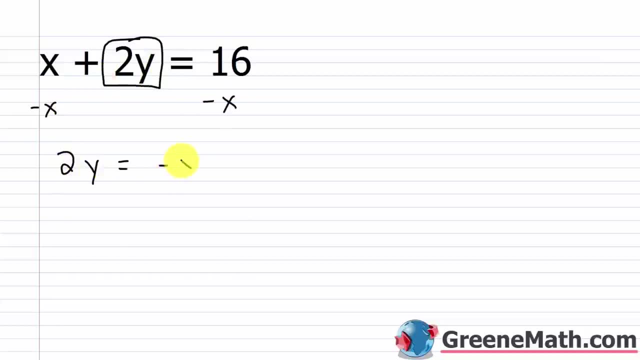 So I would have 2y is equal to negative x plus 16 and then I would divide each side of the equation by 2. 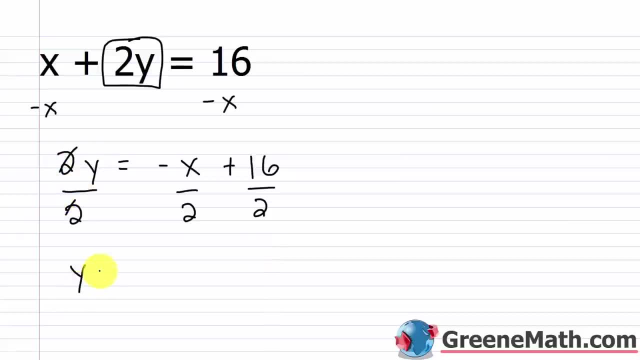 So what would I have? That would cancel. I'd have y is equal to you think about negative x as negative 1 times x. We don't typically write that 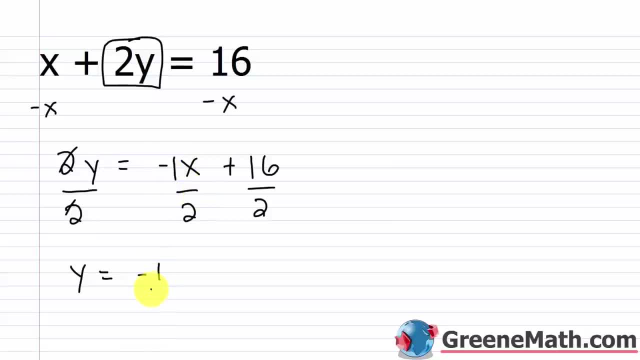 but to make it clear you have negative 1 half times x there. So negative 1 half times x equals 16 over 2 is 8. 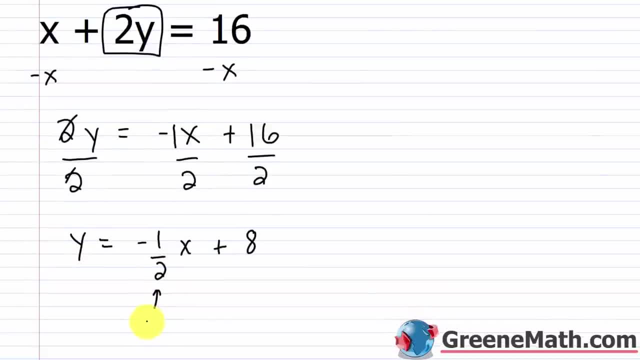 So I have my equation solved for y and now I know that the slope 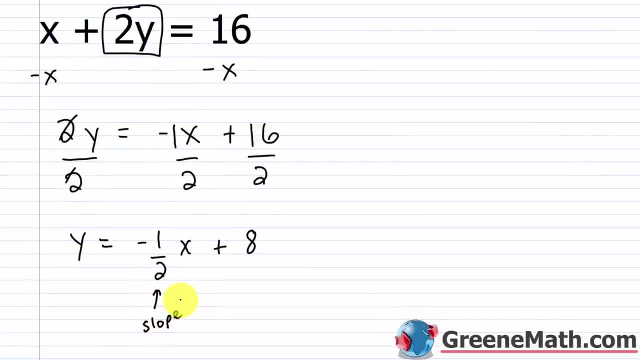 or m is negative 1 half 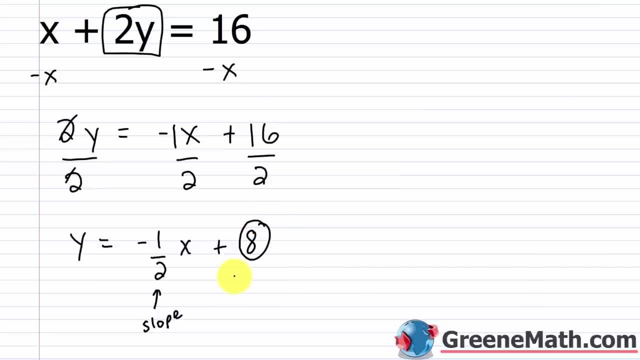 and I know that the y intercept will occur at 0 comma 8. 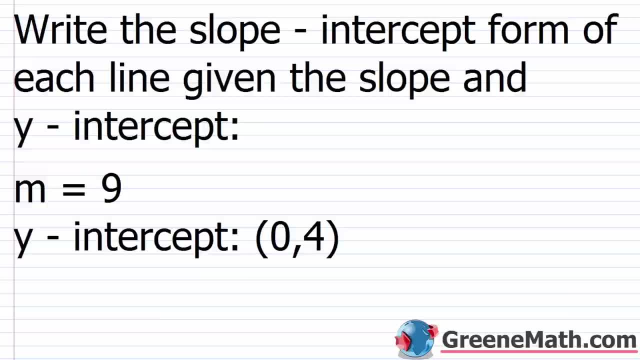 So here's another very common textbook type example. 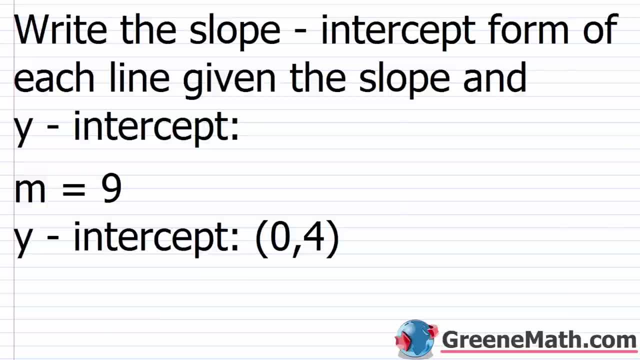 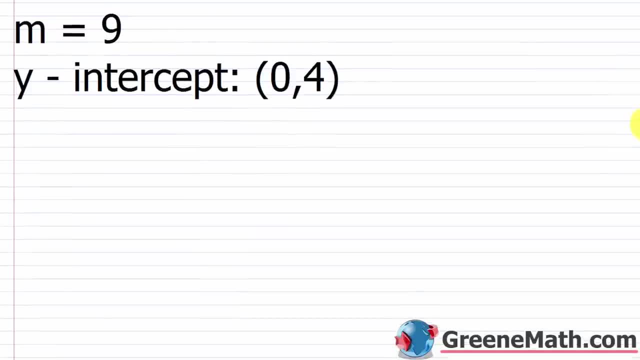 Something you'll probably get on your test. So we want to write the slope intercept form of each line given the slope and y intercept. And we just did this a little while ago. So we have that m equals 9 and again m is standing for slope. So the slope is 9 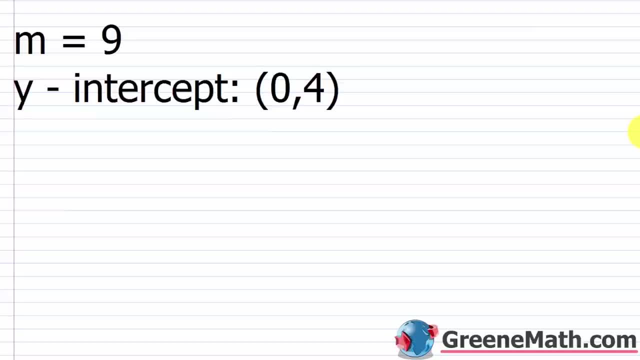 and the y intercept is given as 0 comma 4. 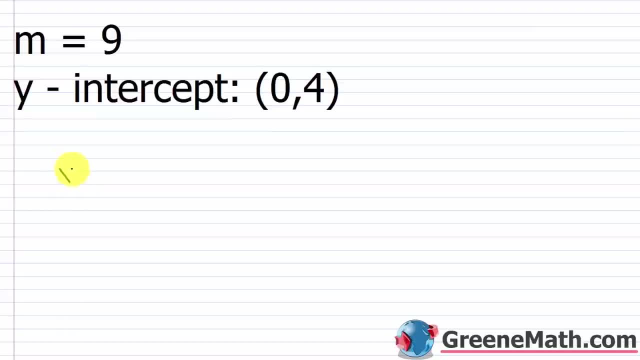 So how do I write the equation? I have y equals mx plus b. If you have a problem like that 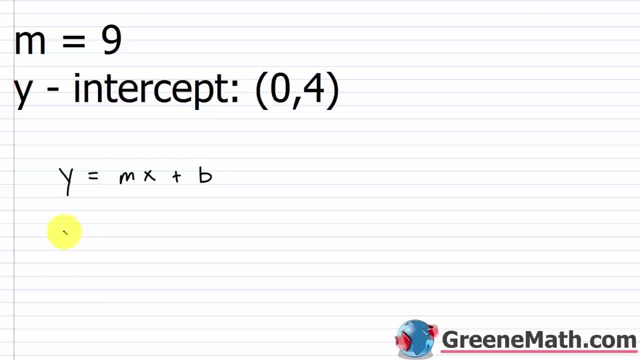 You need to memorize it. And then just duplicate it. 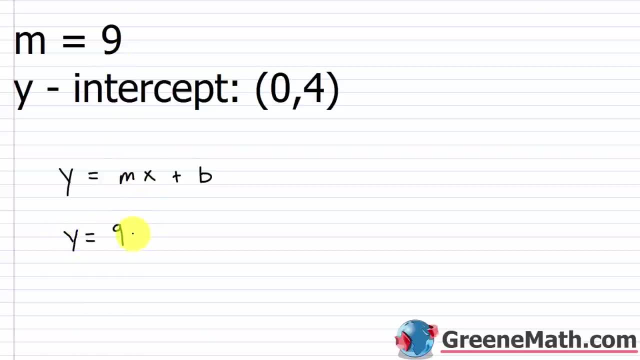 So I have y equals I know what m is, that's 9 then plus b. And again what is b? 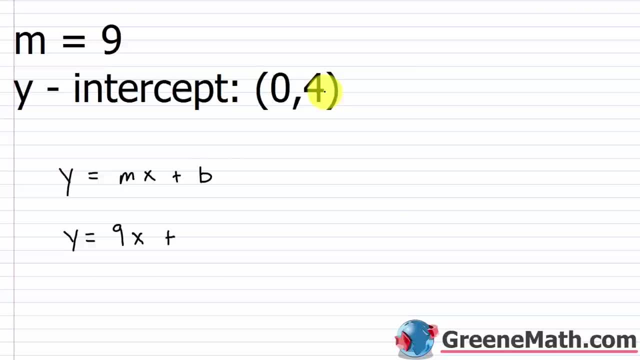 It's the y coordinate when we think about the y intercept. So the y intercept occurs at 0 comma 4 so we just put plus 4. 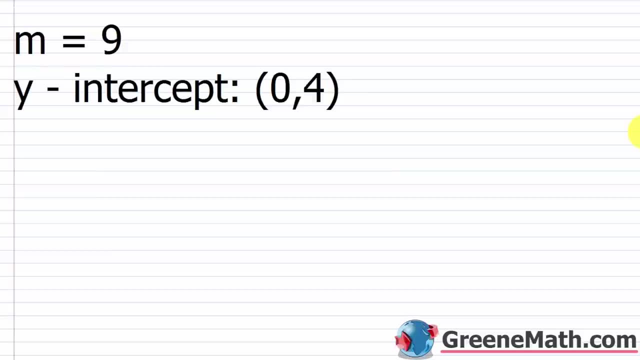 slope. so the slope is 9 and the y-intercept is given as the point 0 comma 4. so how do I write the equation I have: y equals MX plus B. if you have a problem like that, just write that formula out to begin with. you need to. 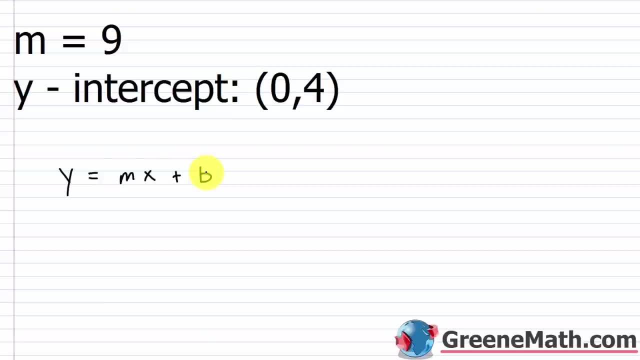 memorize: y equals MX plus B, and then just duplicate it, so I have y equals. I know what M is. that's 9, then times X, then plus B, and again what is B? it's the y-coordinate. when we think about the y-intercept, so the y-intercept occurs at 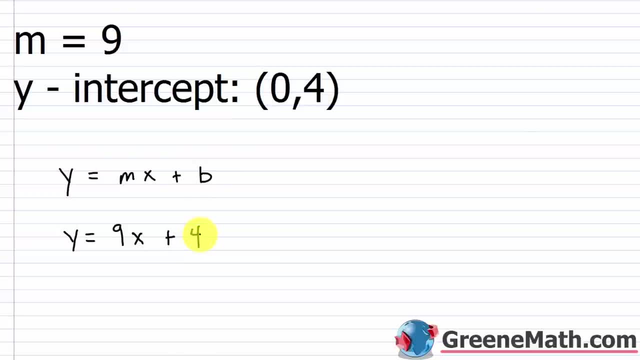 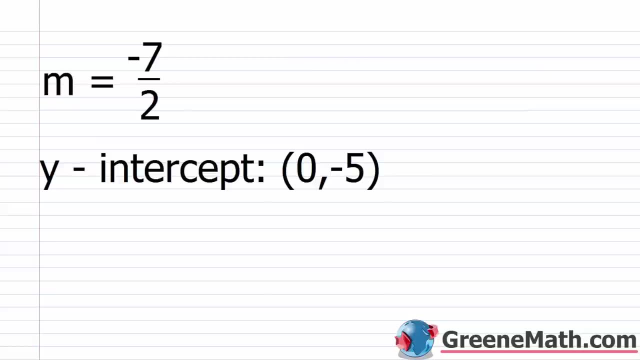 0 comma 4. so we just put plus 4. so y equals 9x plus 4. alright, so the next one I'm given is a slope: M equals negative 7, halves y-intercept occurs at 0 comma negative 5. so again start out by writing that generic formula which is: y equals MX plus. 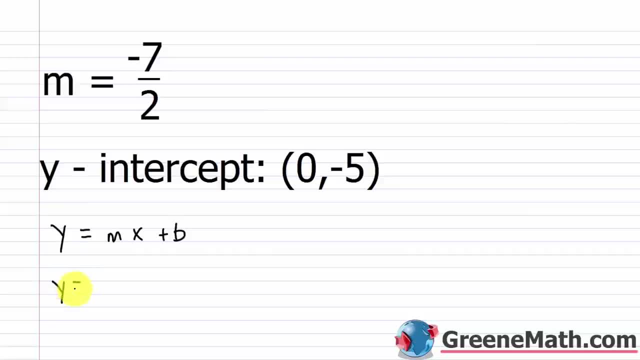 B and just plug in. so y equals my M is negative 7 halves, so negative 7 halves times X and then plus B. so in this case your B is going to be negative 5. so I'm gonna put minus 5. you could also put plus negative 5. either way it's the same. 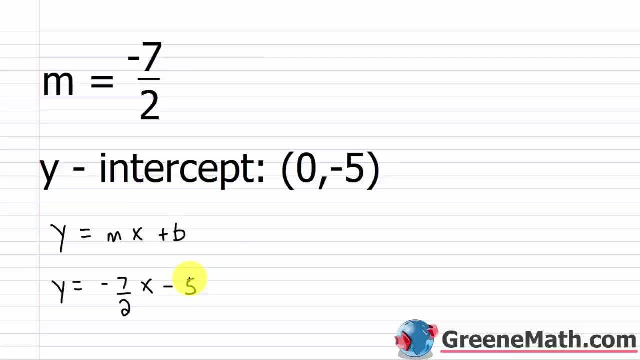 unit both: y equals negative 7 halves X minus 5. all right, what about if M is equal to 5 thirds? okay, so a slope of 5 thirds and a y-intercept that occurs at 0 comma negative 4. so again write your generic formula: y equals MX plus B, so y. 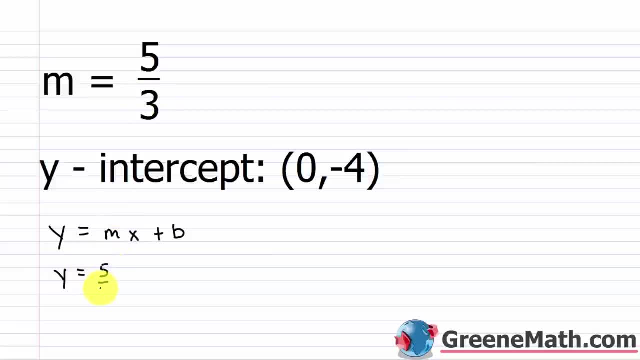 equals what's M, that's 5, 3rds. so 5 3rds times X. and then your B here is going to be negative 4. so again you can put minus four. you can put plus negative four, doesn't matter. So I'm just gonna put minus four. So y: 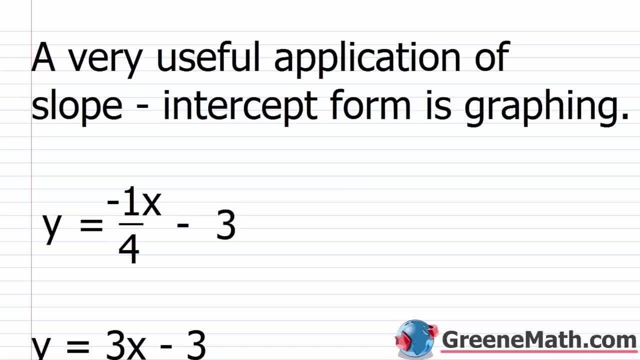 equals five thirds x minus four. Alright, so we're going to kind of wrap up talking about slope intercept form with this last point. So a very useful application of slope intercept form is graphing. This is probably the quickest way to graph a linear equation in two variables. So 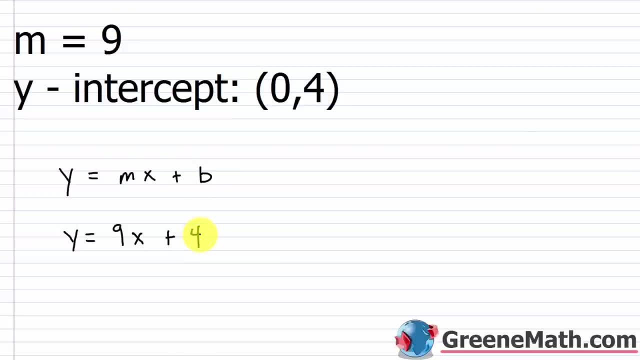 So y equals 9x plus 4. 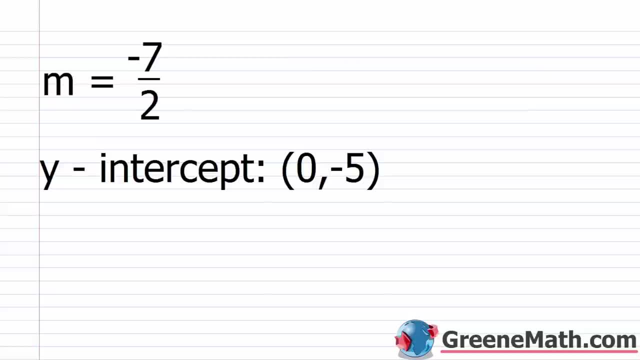 Alright so the next one I'm given is a slope m equals 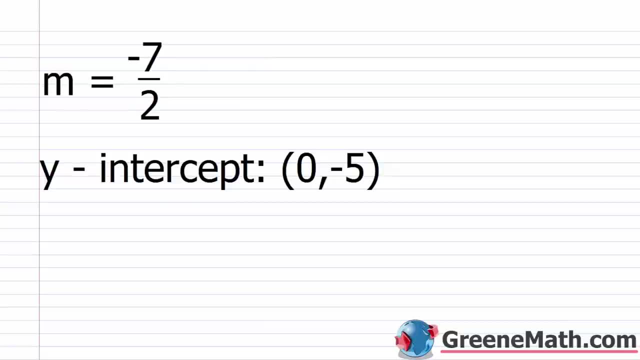 negative 7 halves y intercept occurs at 0 comma negative 5. 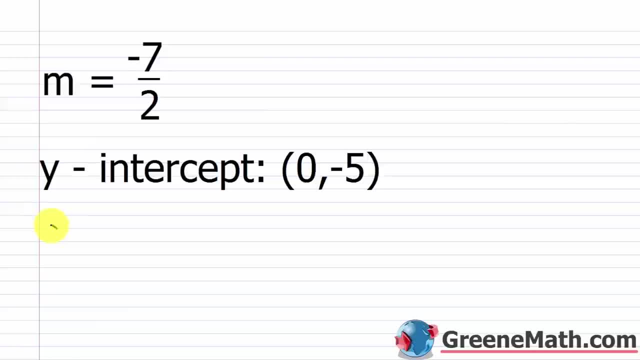 So again start out by writing that generic formula which is y equals mx plus b and just plug in. 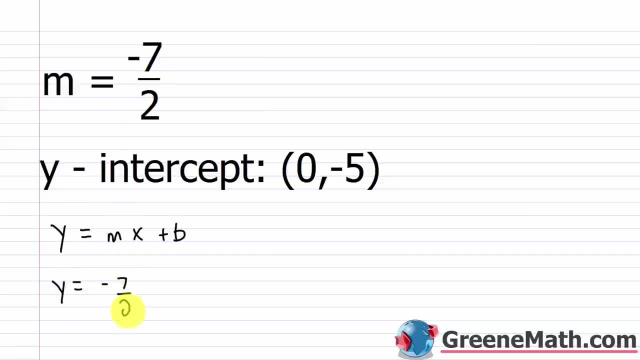 So y equals my m is negative 7 halves times x and then plus b. 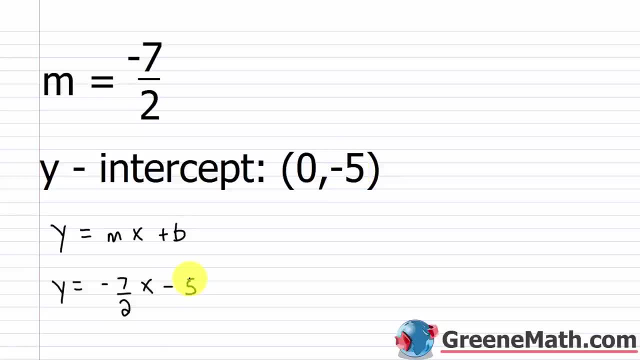 So in this case your b is going to be negative 5. So I'm going to put minus 5 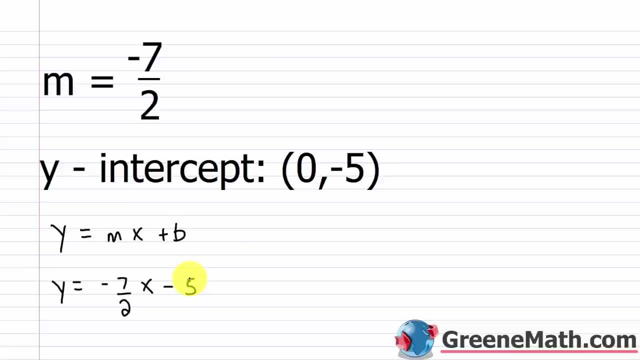 you could also put plus negative 5 either way it's the same. 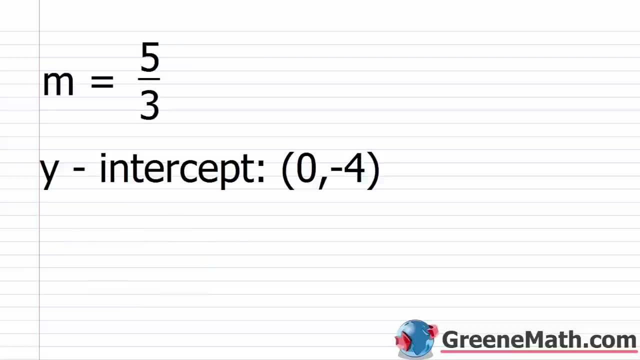 You end up with y equals negative 7 halves x minus 5. 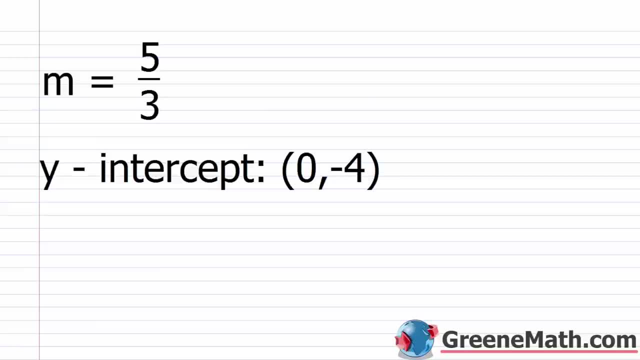 Alright what about if m is equal to 5 thirds so a slope of 5 thirds and a y intercept that occurs at negative 4. 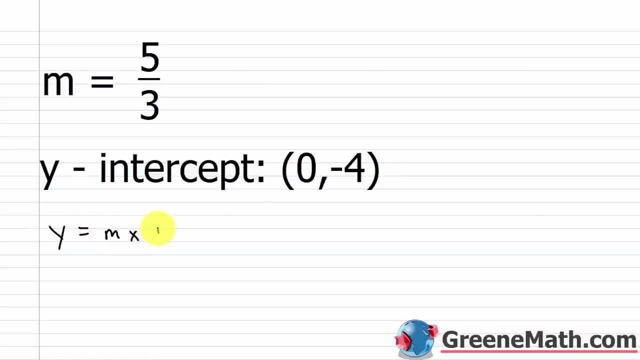 So again write your generic formula y equals mx plus b so y equals what's m that's 5 thirds so 5 thirds times x and then your b here is going to be negative 4. 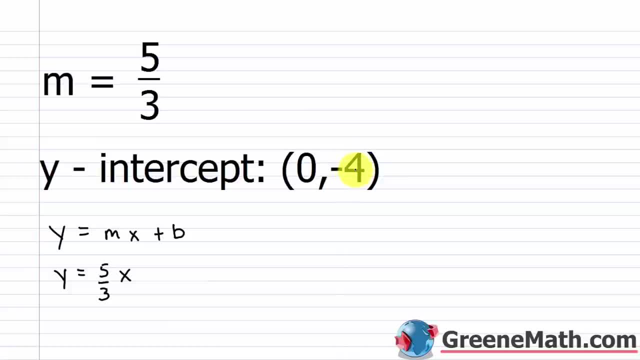 So again you can put minus 4 you can put plus negative 4 doesn't matter so I'm just going to put minus 4. 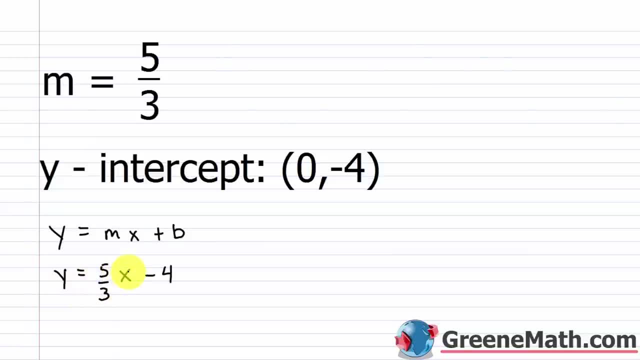 So y equals 5 thirds x minus 4. 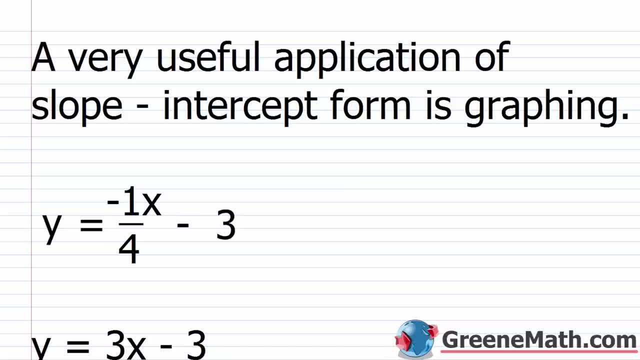 Alright so we're going to kind of wrap up talking about slope intercept form with this last point. So a very useful application of slope intercept form is graphing. 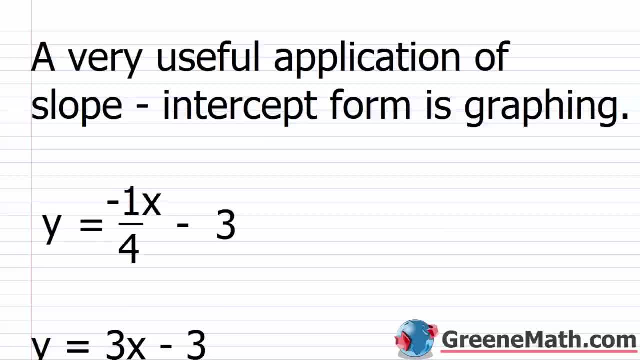 This is probably the quickest way to graph a linear equation in two variables. 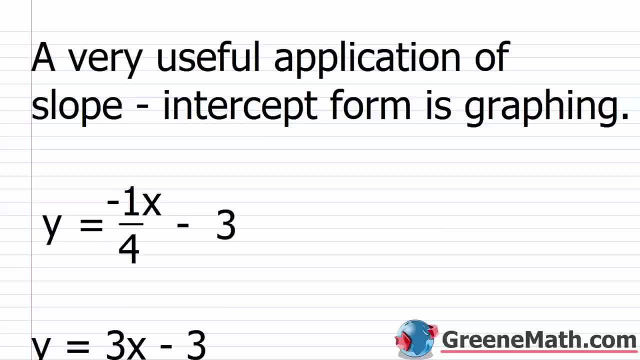 So if we had had this you know a few lessons ago when we first started talking about it you'd be like man this is really 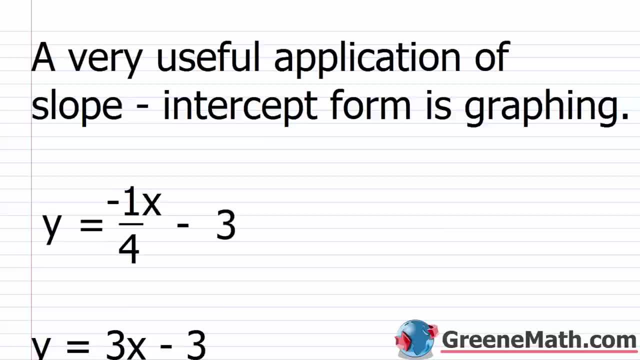 easy. So if you have something in slope intercept form you automatically have the slope and you have a point on the line you have the y intercept. 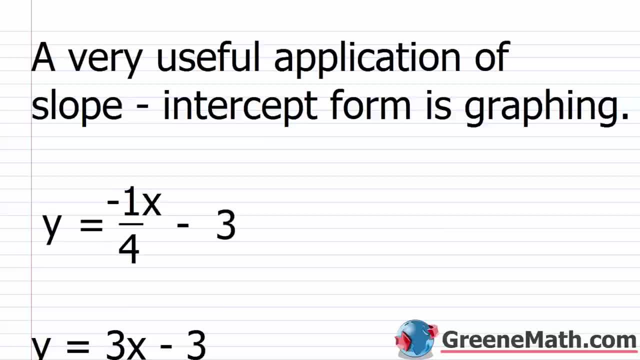 if we'd had this, you know, a few lessons ago, when we first started talking about it. you know, like man, this is really easy. So if you have something in slope intercept form, you automatically have the slope and you have a point on the line, you have the y intercept. 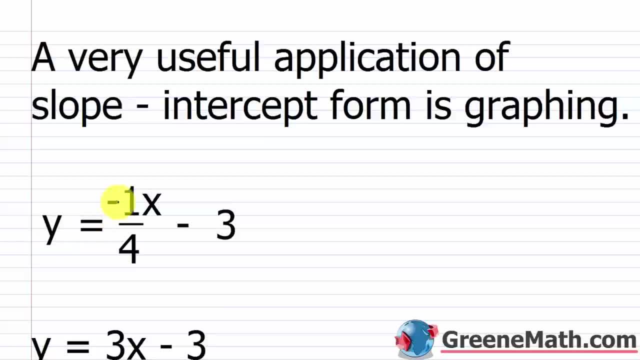 So it's super, super easy to graph it. So if I have y equals negative one fourth, x minus three, I know that the slope m is equal to negative one fourth, And I know that the y intercept, the y intercept, is going to occur at zero comma negative three. So to graph this equation, 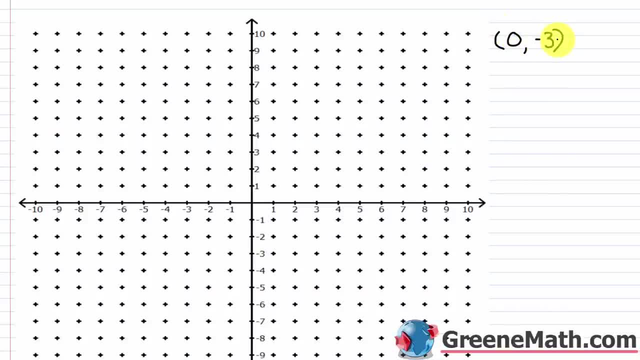 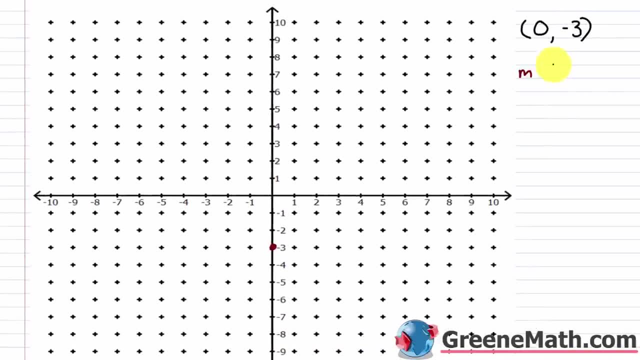 I have that point on the line zero, comma, negative three. that's where I'm going to start Again. that's my y intercept, So that's going to be right here And again. the slope m is negative one. fourth: Now recall when we first started talking about 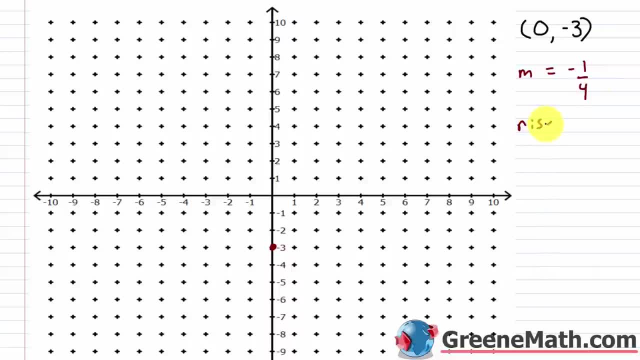 slope. we refer to it as rise over run. So this equals negative one over four. Or you could also think about it as one over negative four. These are the same. Remember, if I have a negative divided by a positive or positive, I'm going to have a negative over negative four. So I'm going 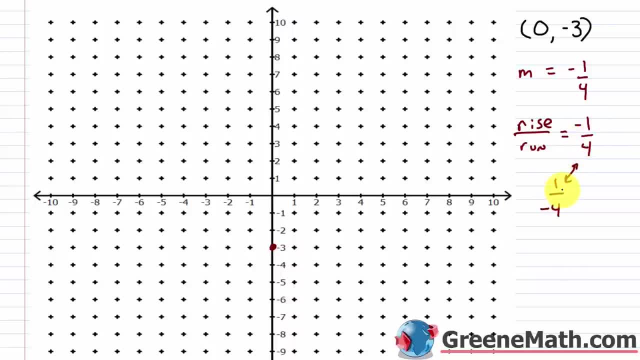 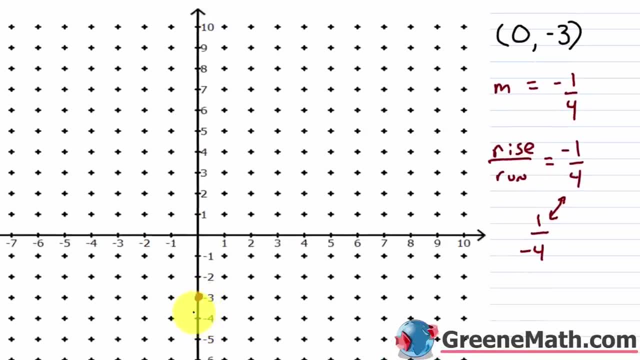 to have a positive divided by a negative: Net, net, net. in the end it's a negative, So you can write that either way. So, starting from this point, I can fall one and go over four. That's rise over run. So if I rise negative one, I'm falling one. If I run four, I'm going to the. 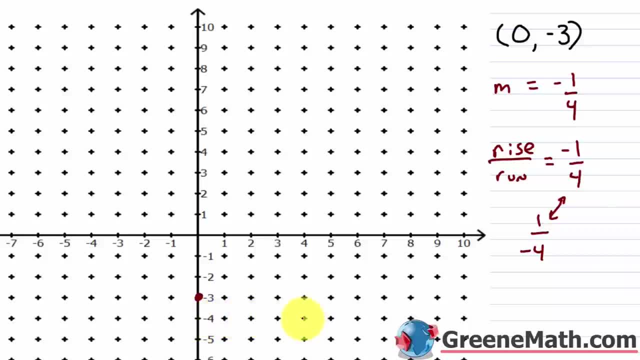 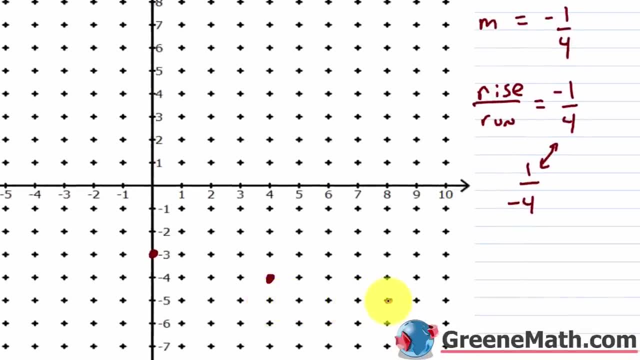 right, four. So I'm going one, two, three, four. So this would be the next point on the line And I'll do that again. We'll fall one over one, two, three, four And you can get some points. 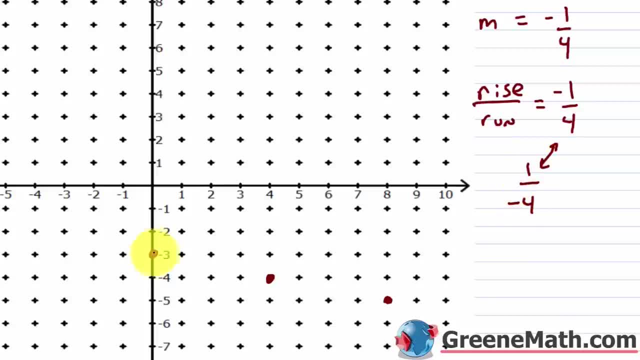 here too, by kind of reversing that and saying, okay, I can also rise one and go to the left four. Right, If I have negative four in the position of run, that means I'm going to the left four. So one, two, three, four. Do that again. Up one over to the left. one, two, three, four. 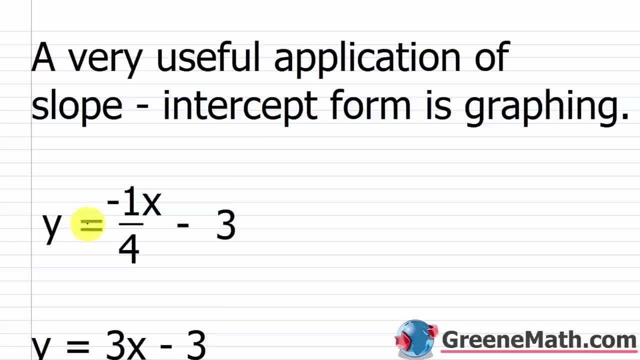 So it's super super easy to graph it. So if I have y equals negative 1 fourth x minus 3 I know that the slope m is equal to negative 1 fourth and I know that the y intercept the y intercept is going to occur at 0 comma negative 3. 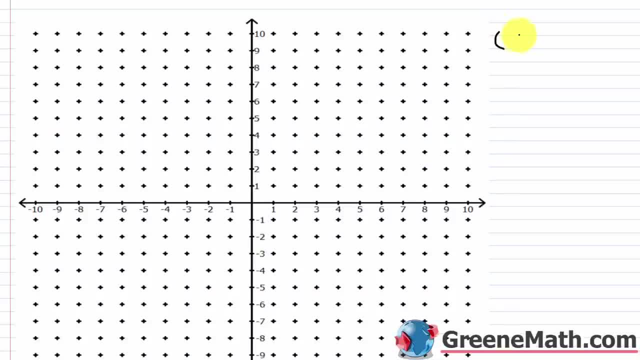 So to graph this equation I have that point on the line 0 comma negative 3 that's where I'm going to start. 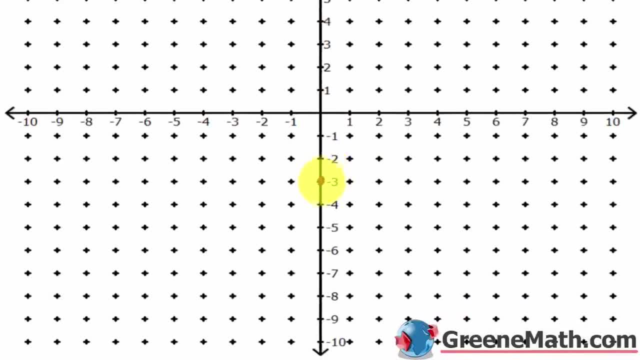 Again that's my y intercept so that's going to be right here. And again 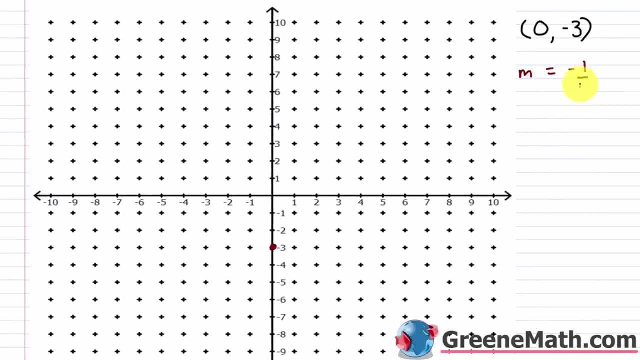 the slope m is negative 1 fourth. 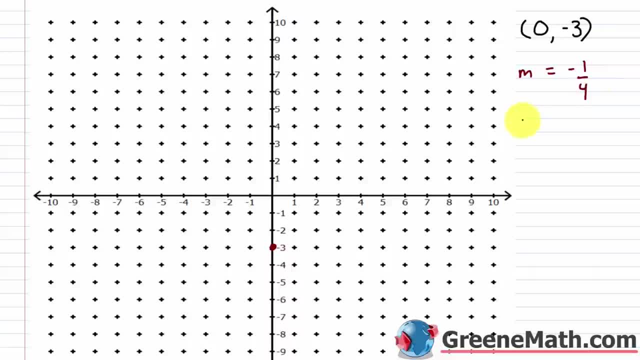 Now recall when we first started talking about slope we referred to it as rise over run. 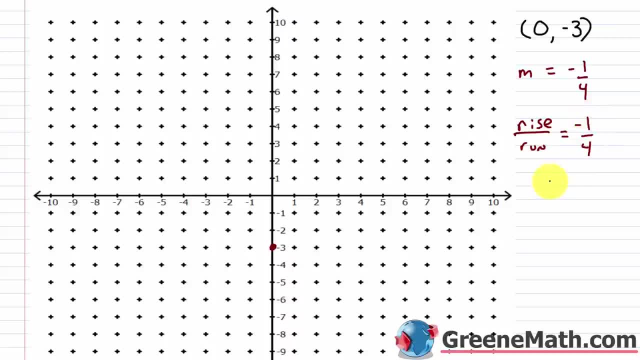 So this equals negative 1 over 4 or you could also think about it as 1 over negative 4. These are the same. Remember if I have a negative divided by a positive or a positive divided by a negative net net net in the end it's a negative. So you can write that either way. So starting from this point I can fall 1 and go over 4. 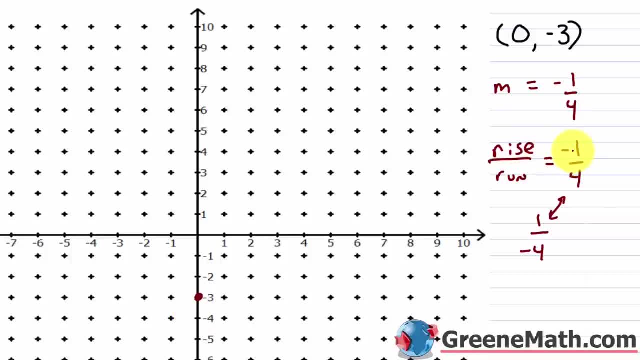 That's rise over run. If I rise negative 1 I'm falling 1. If I run 4 I'm going to the right 4. So I'm going 1, 2, 3, 4. So this would be the next point on the line. 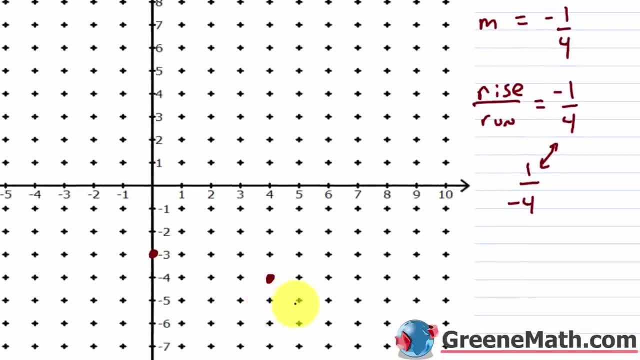 And I'll do that again. Fall 1 over 1, 2, 3, 4. 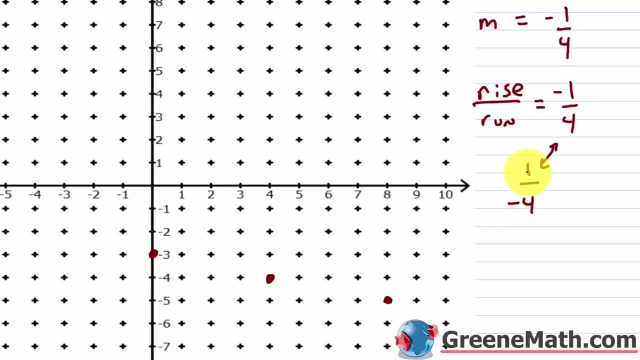 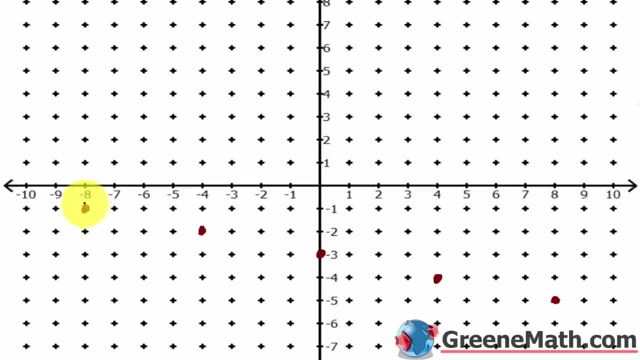 And you can get some points over here too by kind of reversing that and saying okay I can also rise 1 and go to the left 4. If I have negative 4 in the position of run that means I'm going to the left 4. So 1, 2, 3, 4. Do that again. Up 1. Over to the left 1, 2, 3, 4. 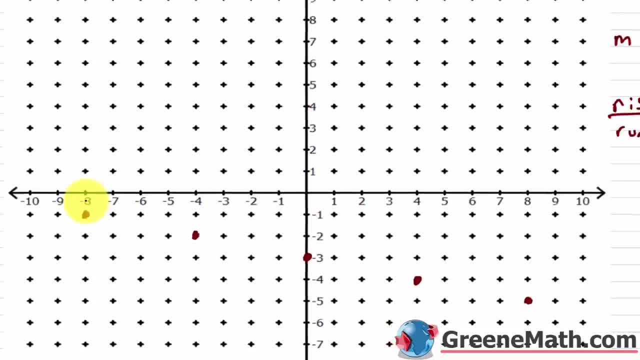 So there are some points. And we just draw a line through them to graph it. 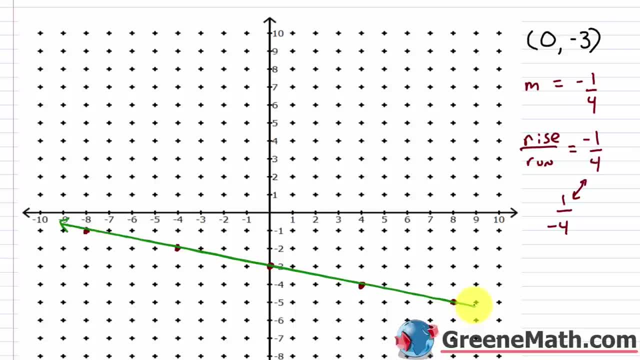 Okay. So now we'll put some arrows at each end. 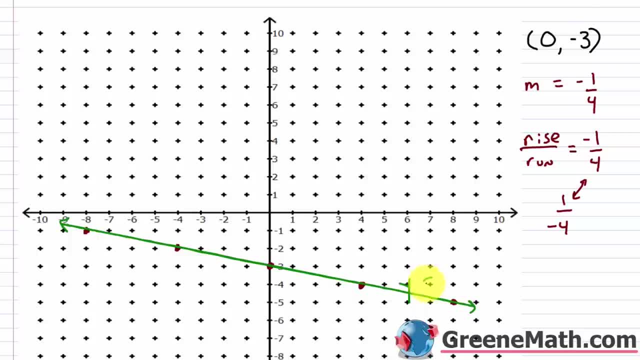 And so this is the equation. Y is equal to negative 1 fourth x minus 3. 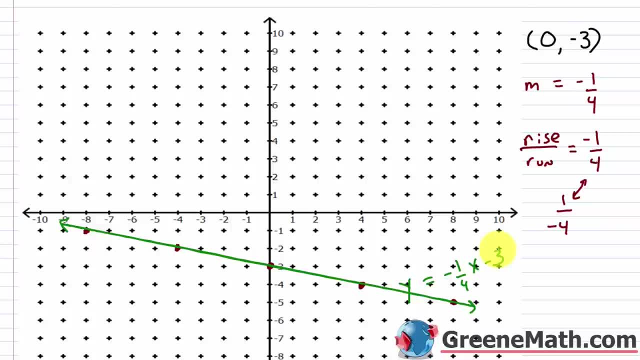 And let's test some of these points just in case you don't believe me. 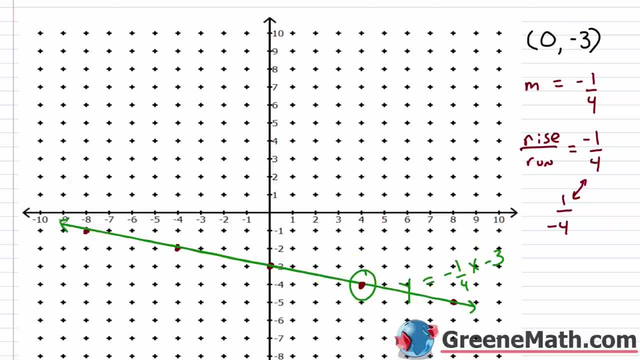 So let's test this point right here which is 4 comma negative 4. 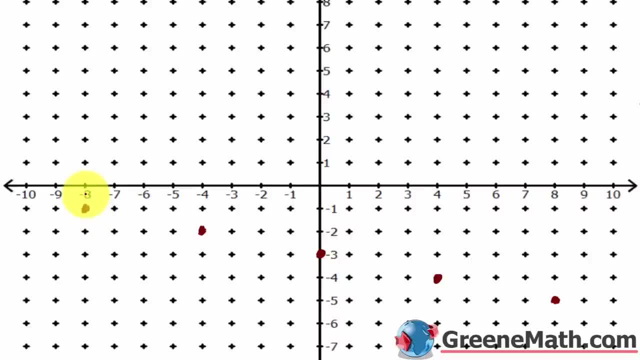 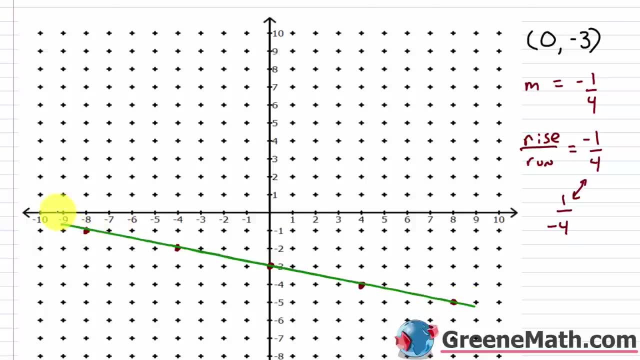 So there are some points And we just draw a line through them to graph it. Okay, So now we'll put some arrows, And so this is the equation: Y is equal to negative one-fourth x minus three. And let's test some of these points, just in case you don't believe me. So 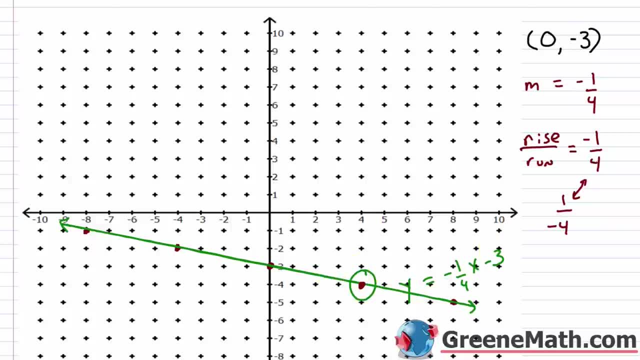 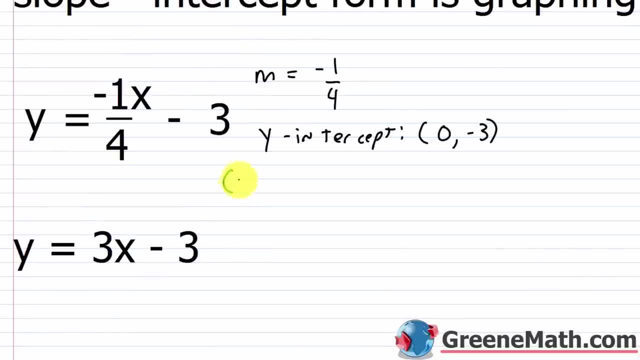 let's test this point right here, which is four comma negative four. So we will go back up here And what I'm going to do is I'm going to test the point four comma negative four. Let's see if that's a solution to this equation. 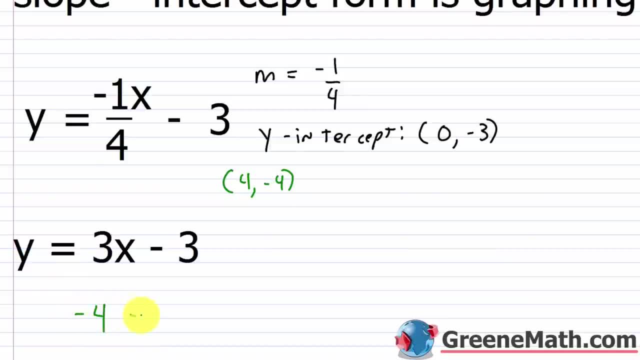 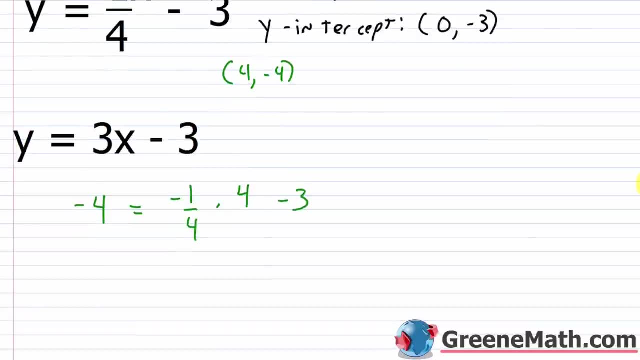 So y in this case is negative four. So negative four is equal to negative one-fourth times positive four minus three, Let's see if each side is equal to the other. So this would cancel with this, leaving me with negative one minus three. Negative one minus three is negative four. 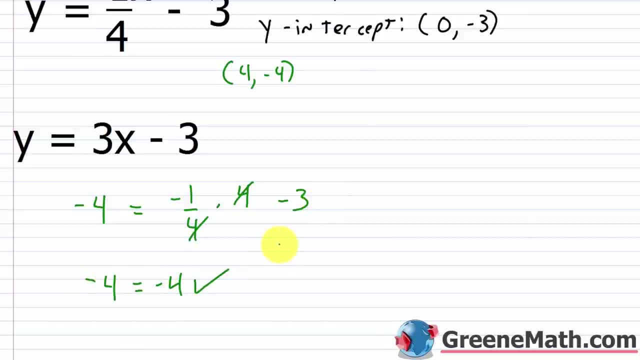 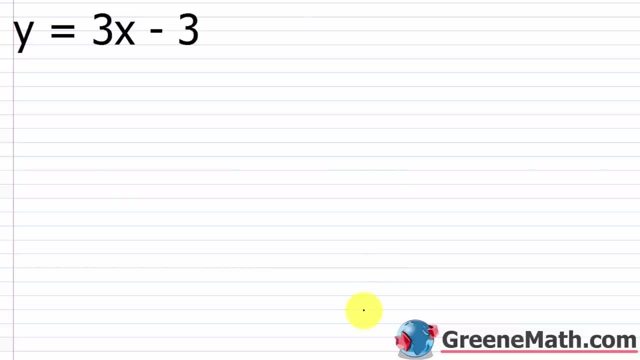 You get negative. four equals negative four. So yeah, that works out All right. So let's try this other one. now. We have y equals three, x minus three. So again it's in slope-intercept form And we know that the slope m is equal to three. Right, This is our. 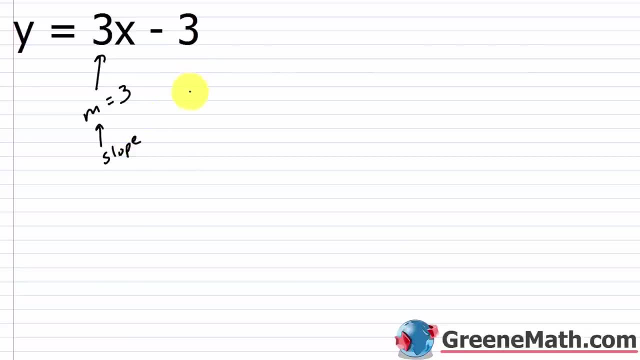 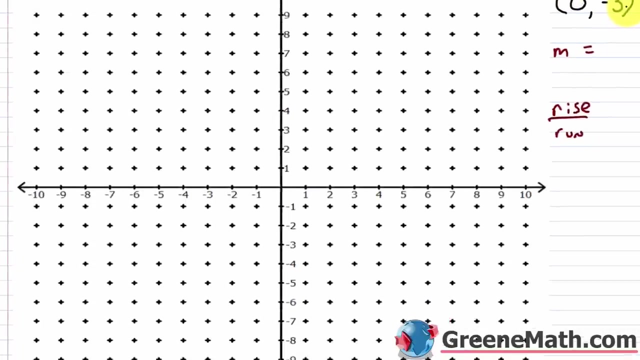 this is our slope. And then we know that the y-intercept occurs. the y-intercept occurs at zero comma negative three. Again, super, super easy to graph this. So our y-intercept is the same as in the last problem: It occurs at zero comma negative three. 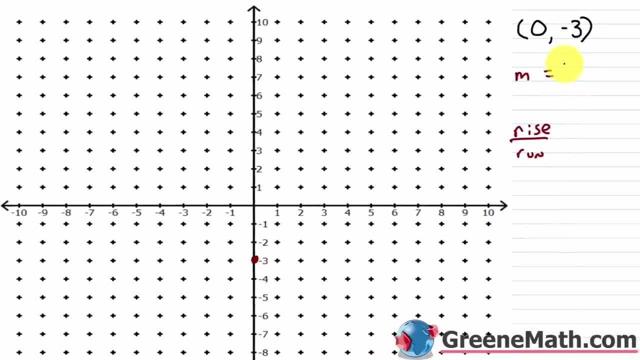 So let's go there. And then our slope was positive three. So the rise over run here. remember, three can be written as a fraction, as three over one. So what that's telling me is that I rise three and I go to the right one. So I start here. I go up one, two, three. 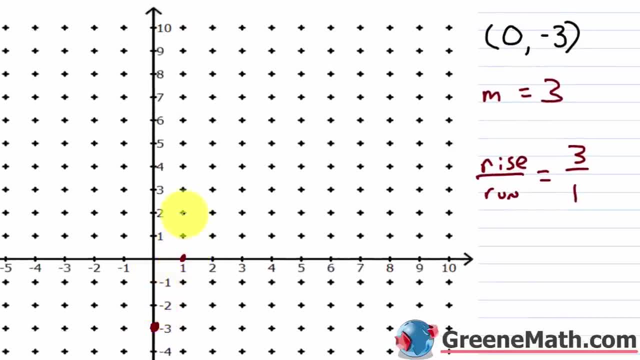 to the right one. That's the point. Rise one, two, three over to the right one. Rise one, two, three over to the right one. You could also think about this as negative three over negative. one Negative over negative is positive, So these two are the same. So I could start here and fall three. 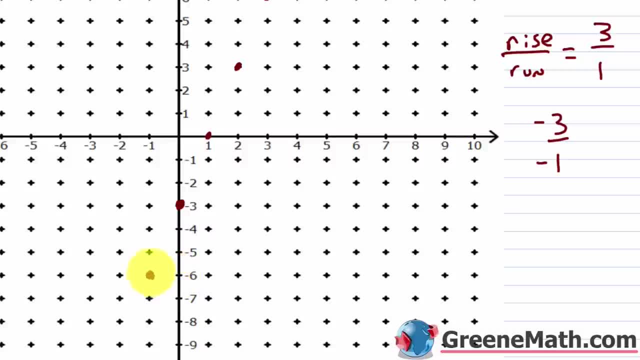 one, two, three Go to the left one, Go to the left one, And if I start from here and follow the original one, Go up one, two, three, Then go the right one over the right one down down half And 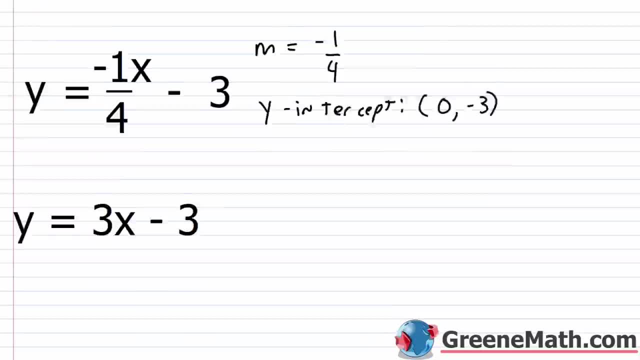 So we will go back up here. And what I'm going to do is I'm going to test the point 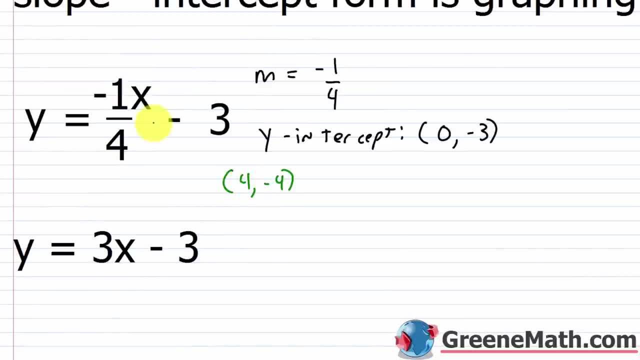 4 comma negative 4. Let's see if that's the solution to this equation. 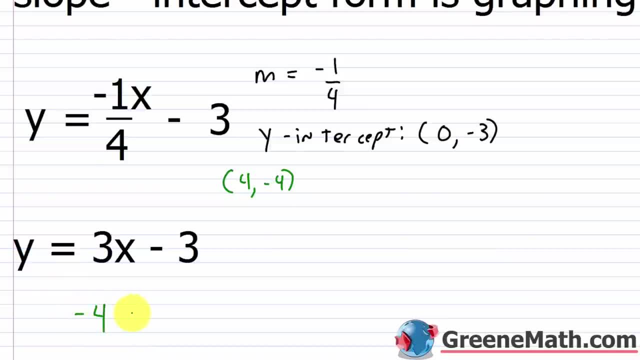 So Y in this case is negative 4. So negative 4 is equal to negative 1 fourth times positive 4 minus 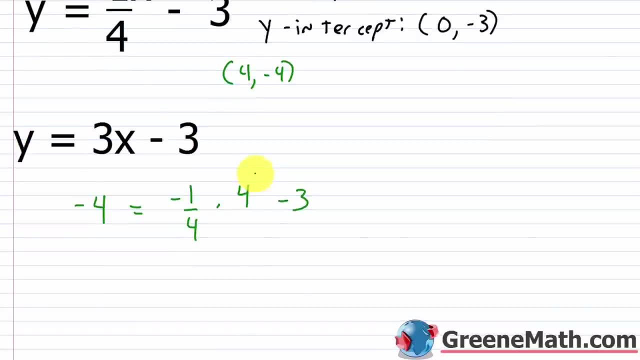 3. Let's see if each side is equal to the other. So this would cancel with this leaving me with negative 1 minus 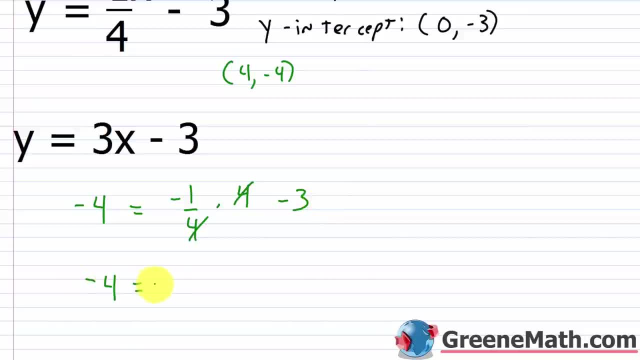 3. Negative 1 minus 3 is negative 4. You get negative 4 equals negative 4. So yeah. That works out. Alright. So let's try this other one now. 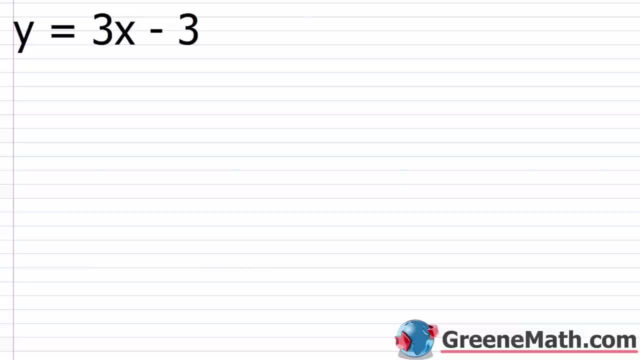 We have Y equals 3x minus 3. So again it's in slope intercept form. And we know that the slope M is equal to 3. This is our slope. 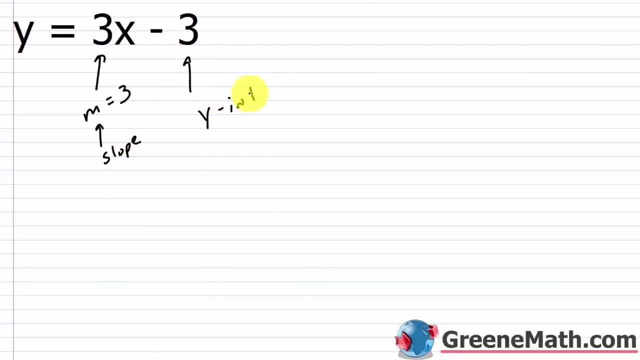 And then we know that the Y intercept occurs the Y intercept occurs 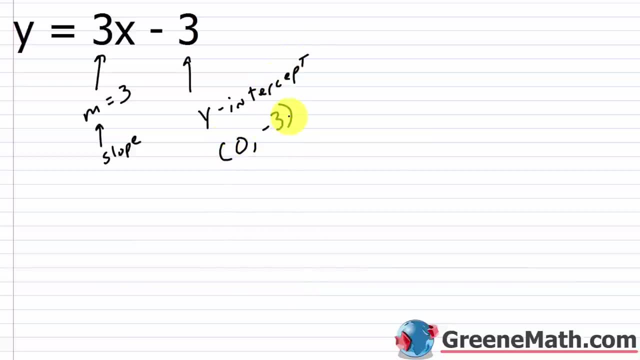 at 0 comma negative 3. Again super super easy to graph this. So our Y intercept is the same as in the last problem. It occurs at 0 comma negative 3. So let's go there. 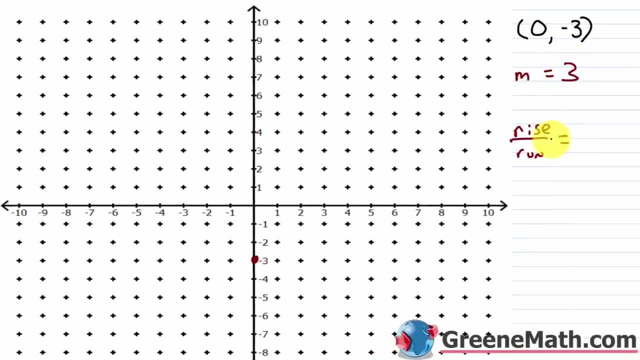 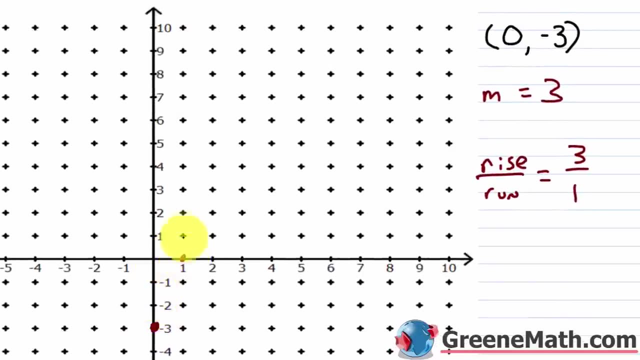 And then our slope was positive 3. So the rise over run here. Remember 3 can be written as a fraction as 3 over 1. So what that's telling me is that I rise 3 and I go to the right 1. So I start here. I go up 1, 2, 3 to the right 1. That's a point. Rise 1, 2, 3 over to the right 1. 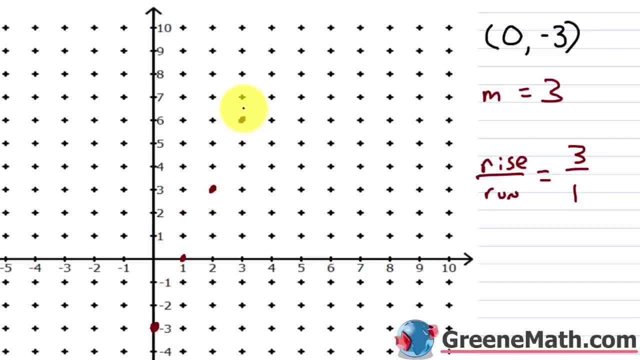 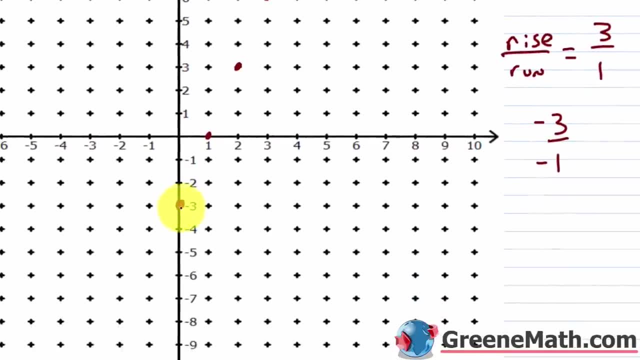 Rise 1, 2, 3 over to the right 1. You could also think about this as negative 3 over negative 1. Negative over negative is positive. So these two are the same. So I could start here and fall 3. 1, 2, 3 go to the left 1. Go to the left 1. And if I start from here and follow the original one 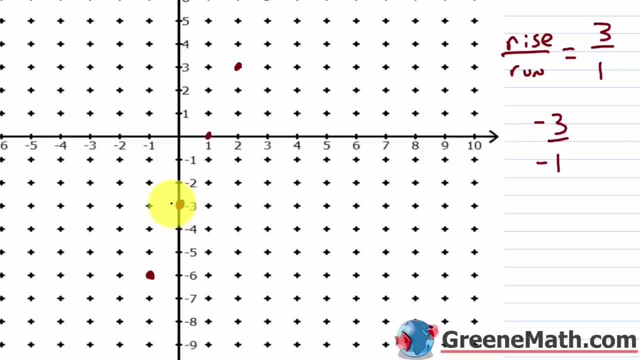 go up 1, 2, 3 to the right 1. I'm back on the line. So let's graph this guy. 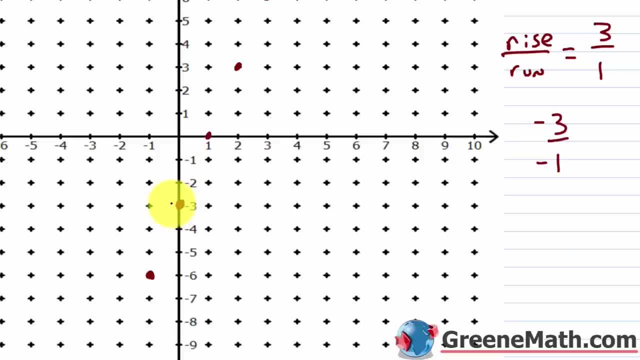 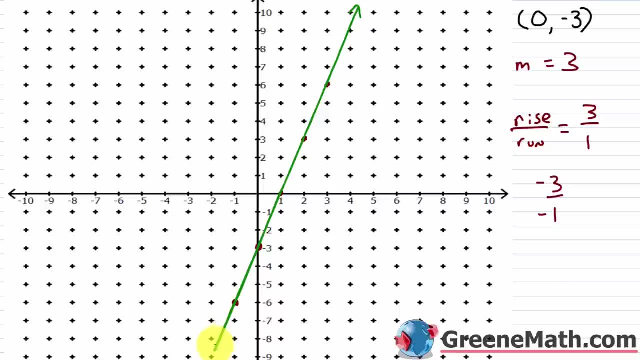 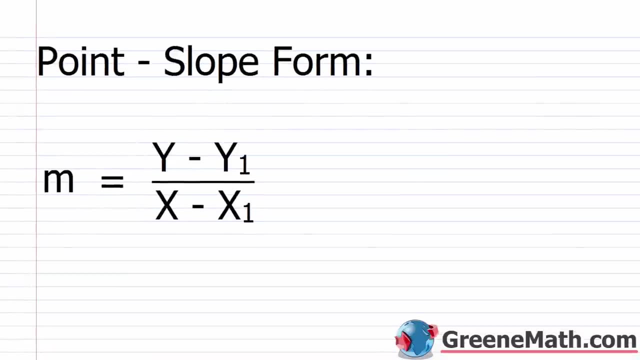 3 to the right 1,. I'm back on the line, So let's graph this guy Again. this is y equals 3x minus 3.. All right, so the next thing we're going to talk about is called point-slope form, So this: 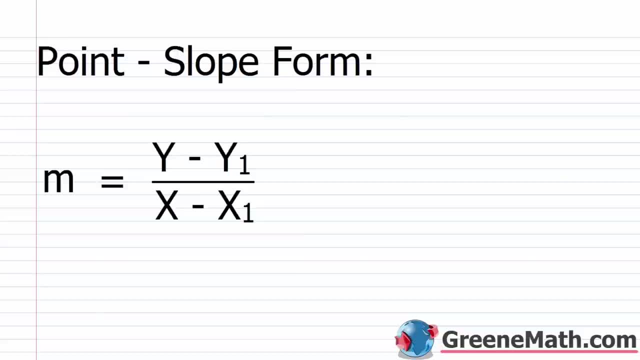 is another thing you talk a lot about in class and it comes from the slope formula. So you have that m. the slope is equal to y minus y sub 1 over x minus x sub 1.. Now there's a little bit. 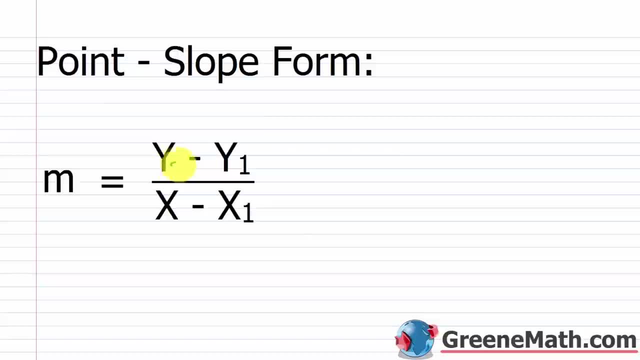 of a difference from the slope formula that you're used to. You're used to seeing y sub 2 minus y sub 1 over x sub 2 minus x sub 1.. Now let me explain why there's a difference. So in a linear equation, 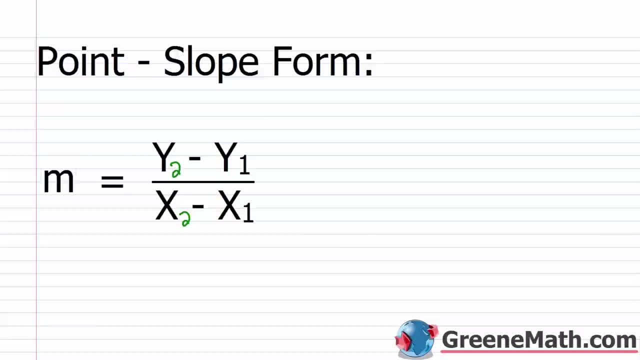 in two variables. when you normally encounter it, you don't have a given x or a y- You don't know what those are. You have something like 5x plus 2y equals 7. So these variables here represent unknowns When we use the slope, 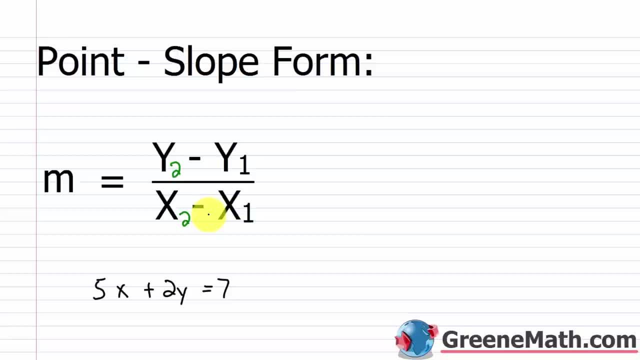 formula like this: we have two points that we're given in most situations. In some that's not the case, But in most situations we're given two points and we plug the given values in right. We plug in the y sub 2,. we plug in the y sub 1,. we plug in the x sub 2, we plug in the x sub 1,. 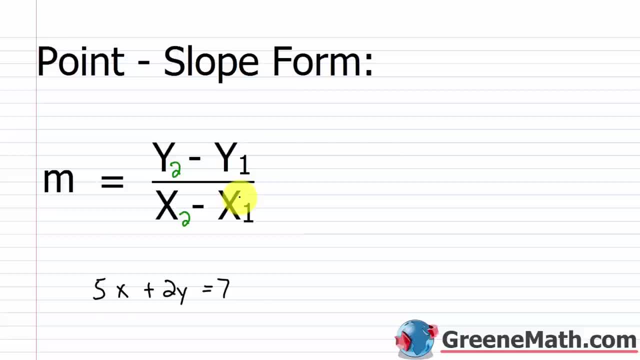 and we do some general arithmetic and we pop out a slope. Well, with point-slope form, what happens is I have a known point, So one known point, and I know the slope, And the slope is known, So this: 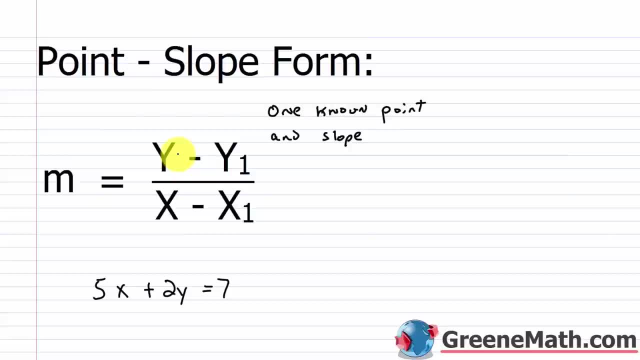 right here, this x and this y that don't have any other notation, that represents the regular x and y that we're thinking of, where we don't know what they are. This x sub 1 and this y sub 1, that's what you're plugging in for with your values from the known point. Okay, so you're. 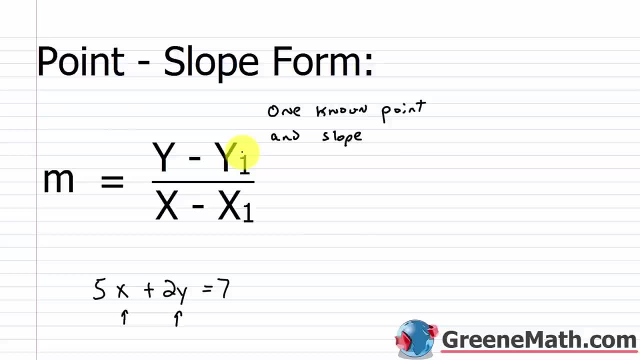 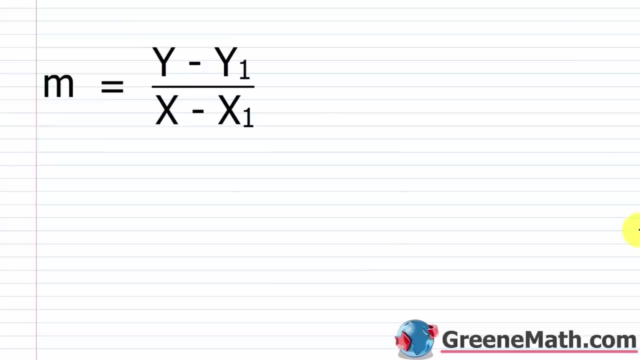 when you have one known point and the slope- And you're going to see some examples where it's not exactly like this, but in most cases you have a known point and you know the slope. So what does point-slope form look like? Well, we just take and multiply both sides. 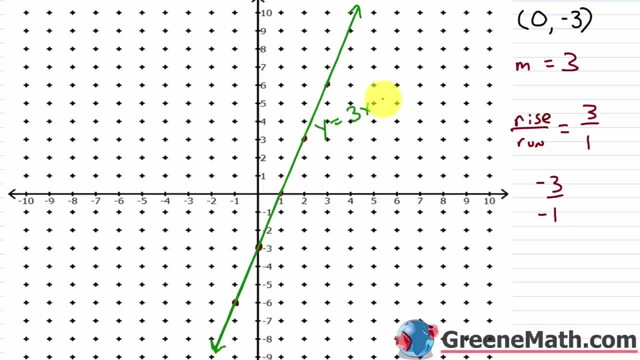 Again, this is y equals 3x minus 3. 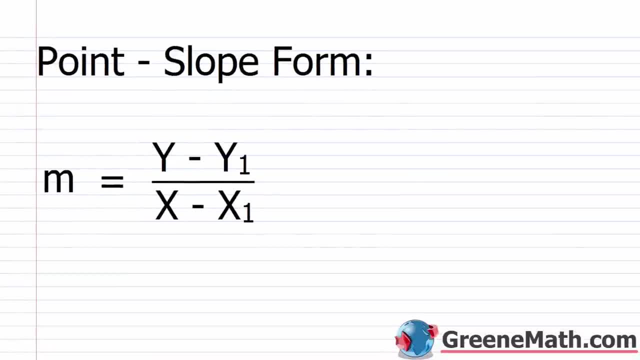 Alright, so the next thing we're going to talk about is called point slope form. 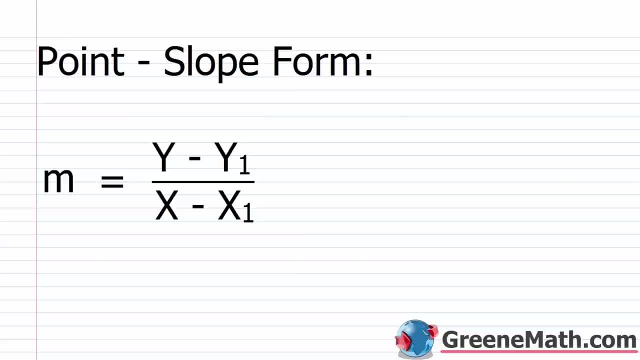 So this is another thing you talk a lot about in class. And it comes from the slope formula. So you have that m, the slope, is equal to y minus y sub 1 over x minus x sub 1. 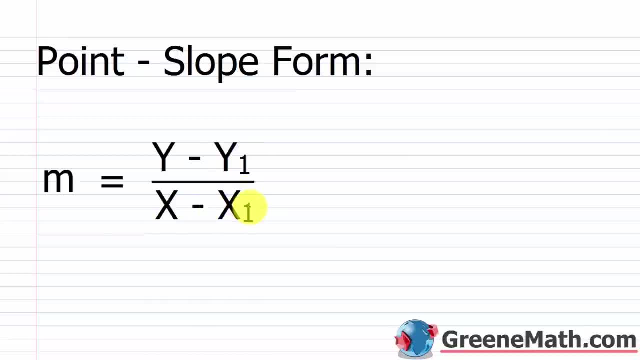 Now, there's a little bit of a difference from the slope formula that you're used to. You're used to seeing y sub 2 minus y sub 1 over x sub 2 minus x sub 1. Now, let me explain why there's a difference. 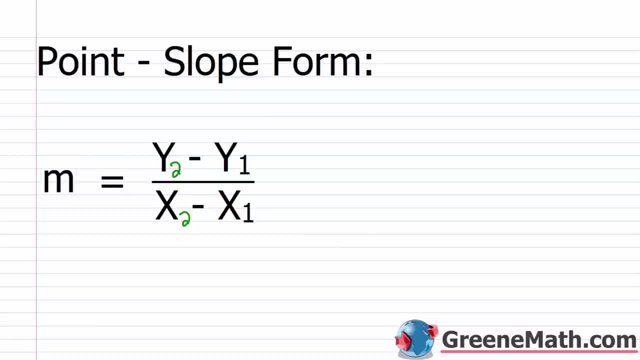 So, in a linear equation in two variables, when you normally encounter it, you don't have a given x or a y. You don't know what those are. You have something like 5x plus 2y equals 7. 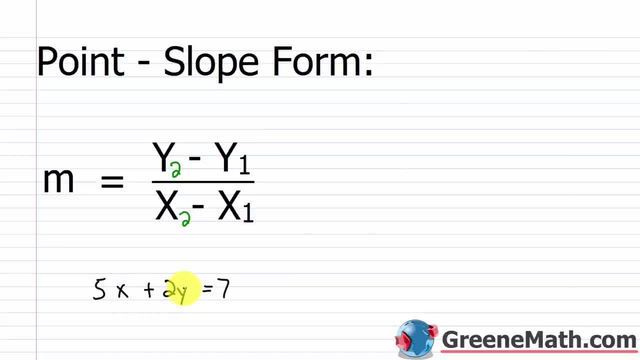 So these variables here represent unknowns. When we use the slope formula like this, we have two points that we're given in most situations. In some, that's not the case. But in most situations, we're given two points. And we plug the given value in, right? We plug in the y sub 2, we plug in the y sub 1, we plug in the x sub 2, we plug in the x sub 1, and we do some general arithmetic and we pop out a slope. 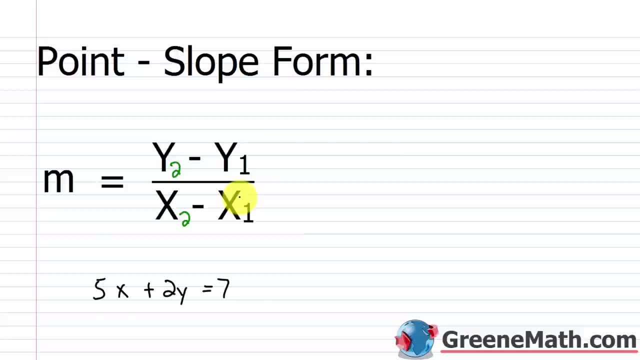 Well, with point-slope form, what happens is, I have a known point. So, one known point and I know the slope. 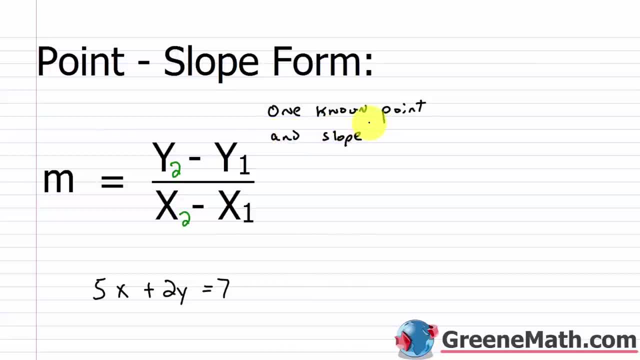 And the slope is known. So this right here, this x and this y that don't have any other notation 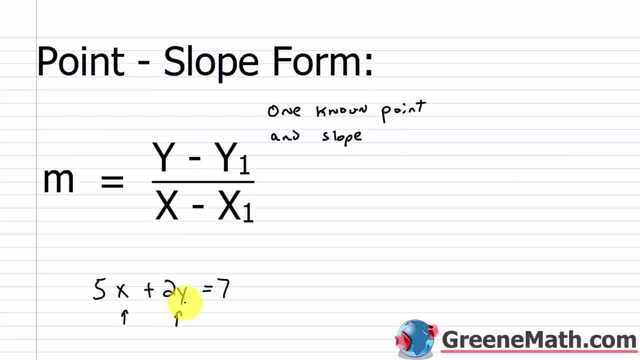 that represents the regular x and y that we're thinking of where we don't know what they are. This x sub 1 and this y sub 1, that's what you're plugging in for with your values from the 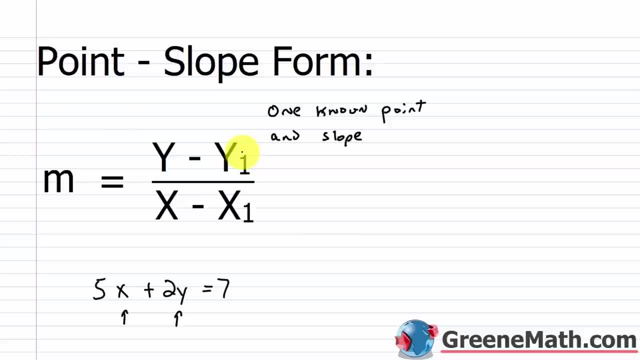 known point. Okay, so you're using point-slope form when you have one known point and the slope. 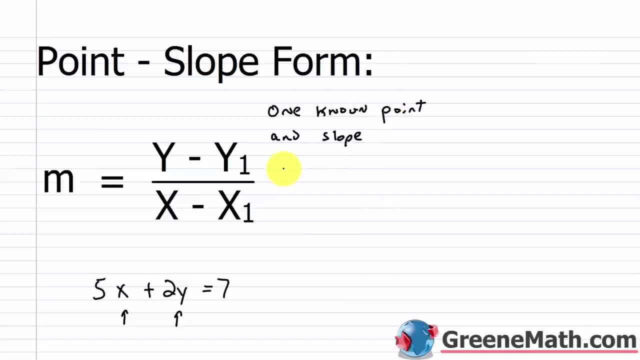 And you're going to see some examples where it's not exactly like this, but in most cases you have a known point 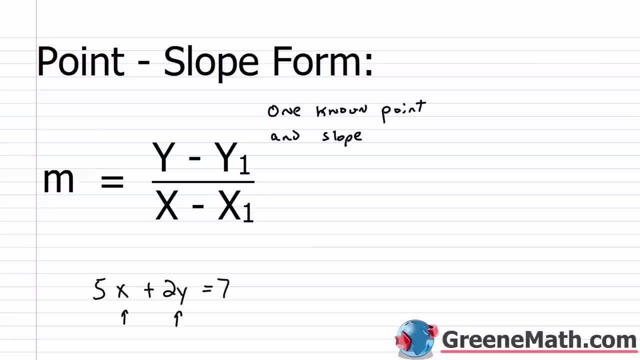 and you know the slope. So, what does point-slope form look like? 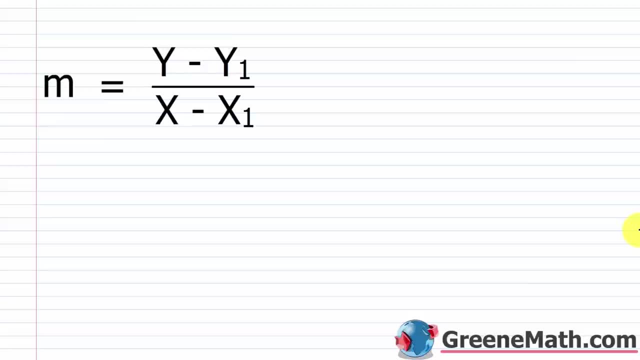 Well, we just take and multiply both sides of the equation by this quantity x minus x sub 1. 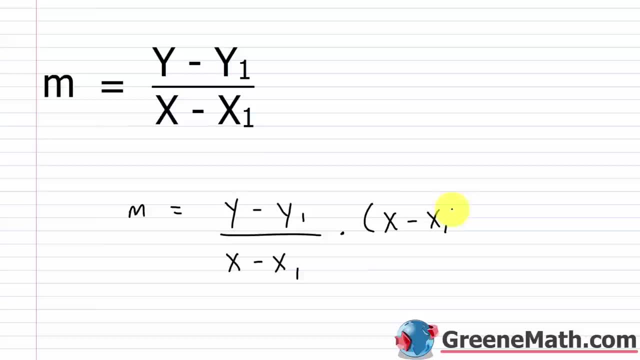 So I'll multiply this over here. And what's going to happen is this is going to cancel with this. It's the same thing divided by itself. So that's going to cancel out. And it's going to be over here x minus x sub 1. Remember to use parentheses. So I can erase this at this point. I can erase this at this point. 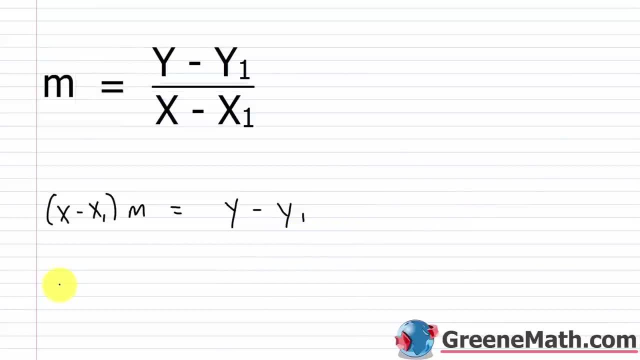 Now it looks a little different in your textbook. In your textbook it's going to look like this. y minus y sub 1 is equal to m times the quantity x minus x sub 1. And you can write it like that. It doesn't matter. I can take this and move it over to the left and take this and move it over to the right. I can put the m out in front. Really all they did was just rewrite it. Nothing is different. 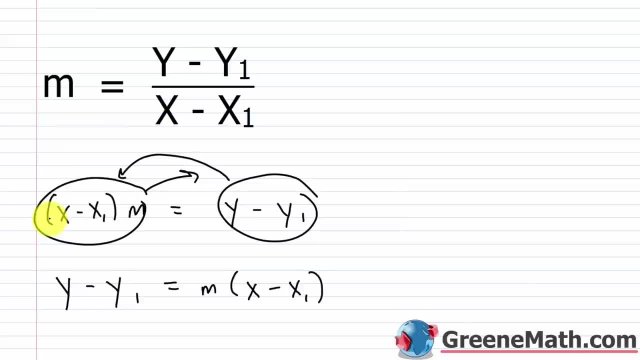 So you need to realize that immediately. So that's where point-slope form comes from. 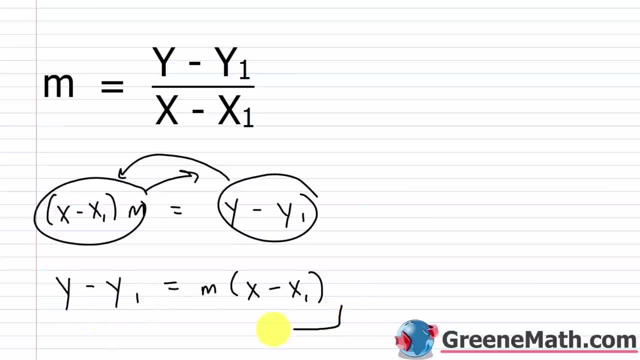 So once you memorize this kind of generic formula here, you're basically ready to go. 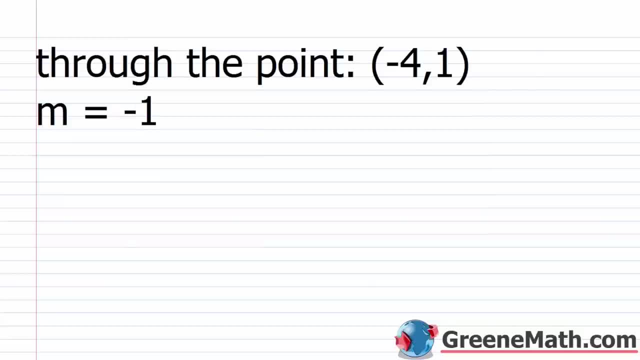 So let's look at an example. So we have a point and we know the slope. So we're going to use our point-slope formula. So we have through the point negative 4 comma 1 with a slope of negative 1. 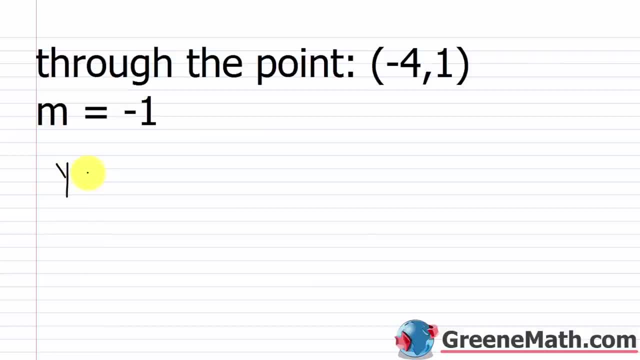 So if I have my point-slope formula y minus y sub 1 is equal to m times the quantity x minus x sub 1. 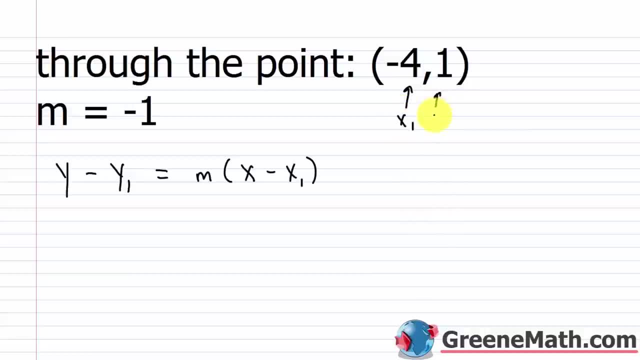 This known point, we label that as x sub 1 y sub 1. 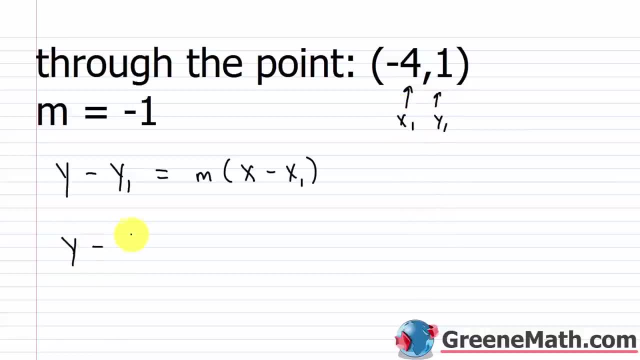 So I'm just plugging in. So I have y minus 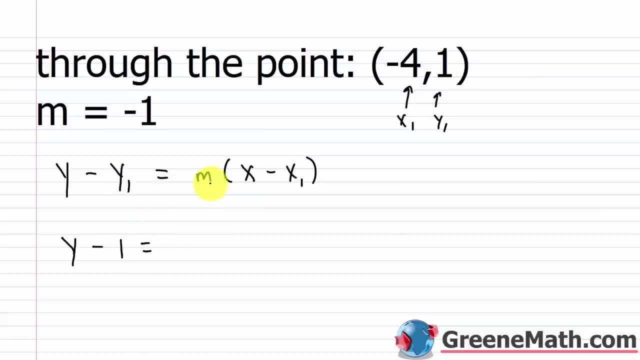 my y sub 1 is 1 equals my m is negative 1 times the quantity x minus x sub 1. We know that's negative 4. 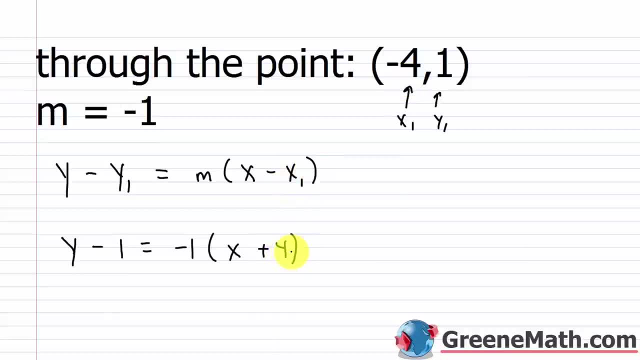 Minus the negative 4 is plus 4. And so once you have this, this is point-slope form. 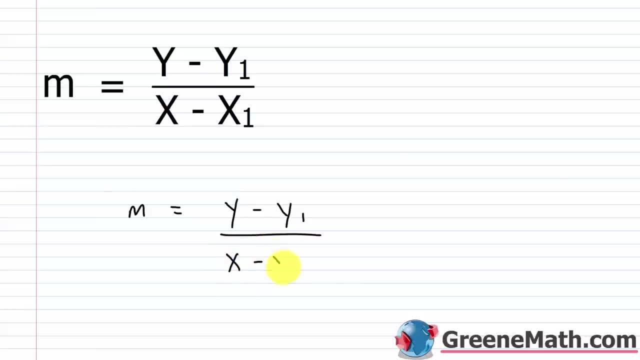 of the equation by this quantity: x minus x sub 1.. So I'll multiply this over here And what's going to happen is this is going to cancel. with this right, It's the same thing divided by itself. So that's going to cancel out And it's going to be over here: x minus x sub 1.. 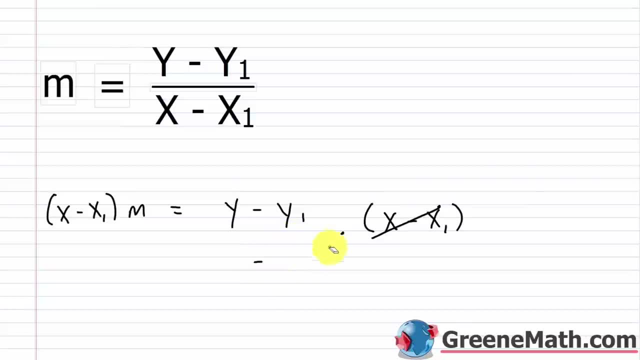 Remember to use parentheses, So I can erase this at this point. I can erase this at this point. Now it looks a little different in your textbook. In your textbook it's going to look like this: y minus y sub 1 is equal to m times the quantity x minus x sub 1.. And you can write it like that. 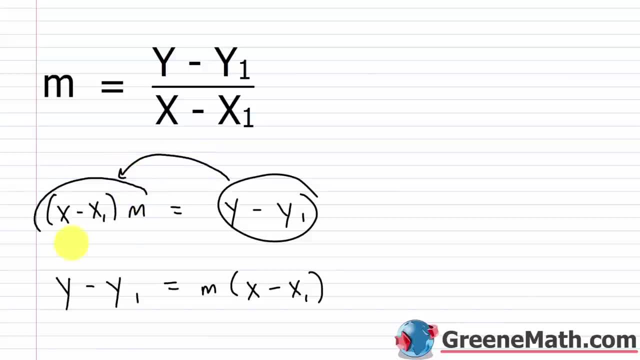 It doesn't matter, I can take this and move it over to the left, and take this and move it over to the right. I can put the m out in front. Really, all they did was just rewrite it. Nothing is different, right? So you need to realize that immediately. So that's where point-slope form comes from. 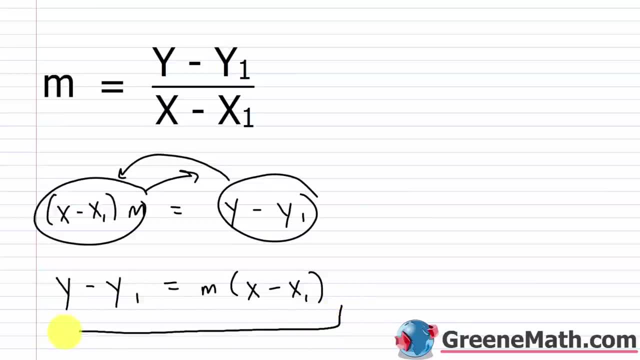 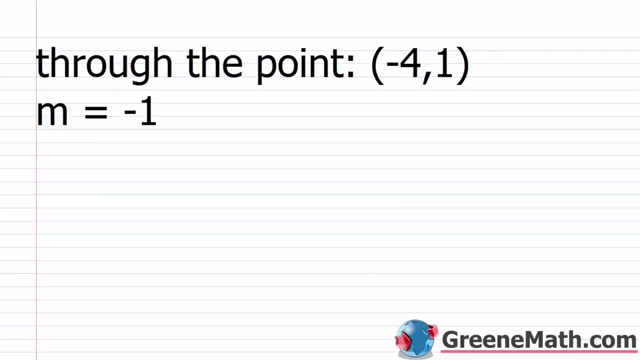 So once you memorize this kind of generic formula here, you're basically ready to go. So let's look at an example. So we have a point and we know the slope, So we're going to use our point-slope formula. So we have, through the point, negative 4, comma 1, with a slope of 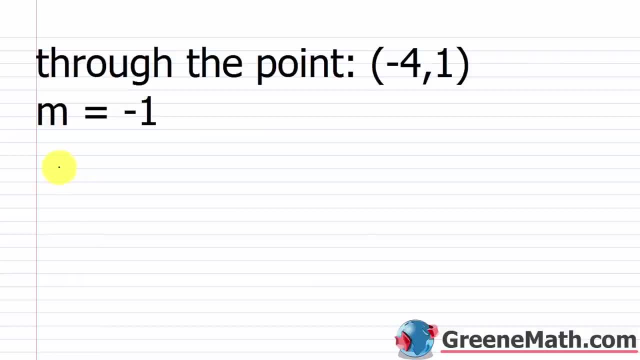 negative 1.. So if I have my point-slope formula y minus y sub 1 is equal to m times the quantity x minus x sub 1.. This known point. we label that as x sub 1, y sub 1.. So I'm just plugging in. So I 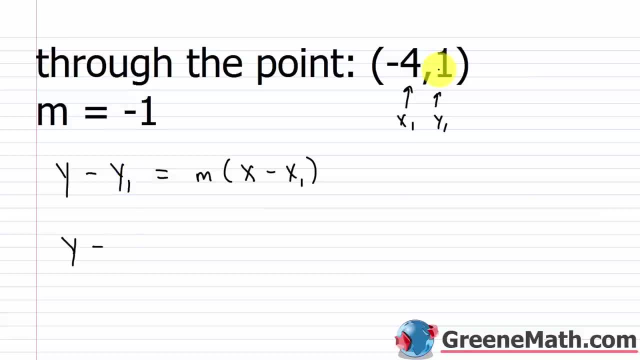 have y minus, my y sub 1 is 1 equals my m is negative 1 times the quantity x minus x sub 1.. We know that's negative 4.. Minus the negative 4 is plus, And so once you have this, this is point-slope form In every situation they're going to want. 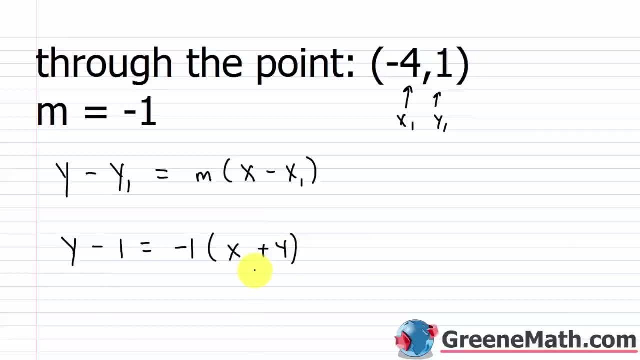 you to solve it for y and put it in slope-intercept form. If the book says, write it in point-slope form, you've done that. This is point-slope form, So you would be done right, Because you've mirrored this right here. That's the same right. I've plugged in for m. I've plugged in for x: sub. 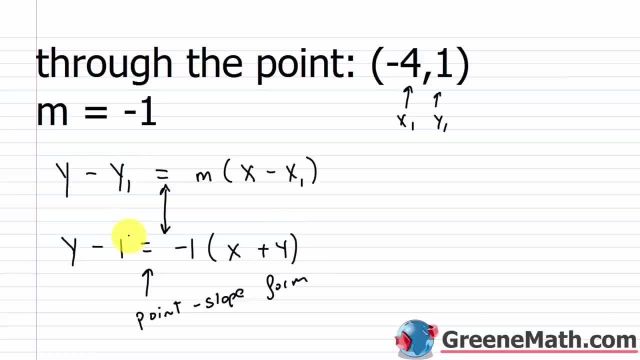 1, and I've plugged in for y sub 1.. So I've done my job, But in most cases they want you to solve it for y sub 1.. So I've done my job, But in most cases they want you to solve it for y sub 1.. 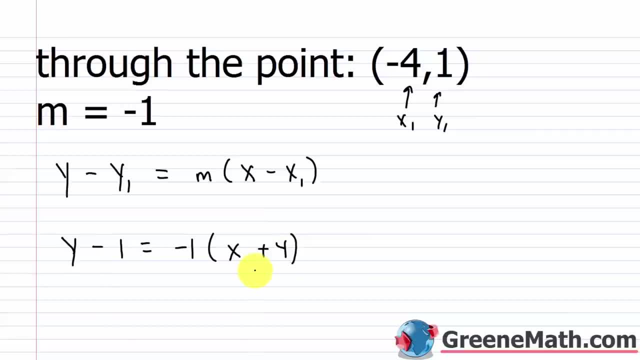 In every situation, they're going to want you to solve it for y and put it in slope intercept form. If the book says write it in point-slope form, you've done that. This is point slope form. So you would be done. 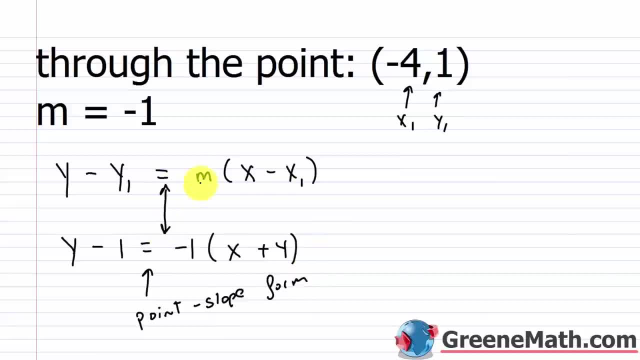 Because you've mirrored this right here. That's the same. I've plugged in 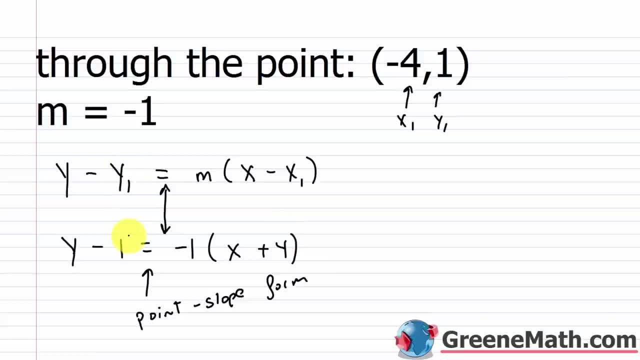 for m, I've plugged in for x sub 1, and I've plugged in for y sub 1. 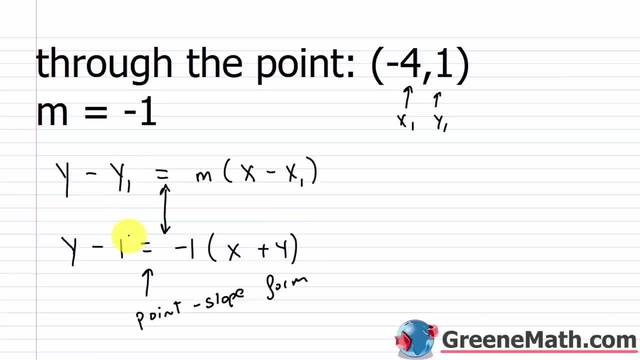 So I've done my job. But in most cases, they want you to solve it for y 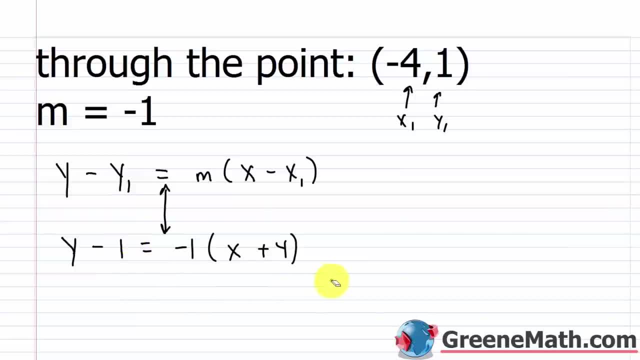 and put it in slope intercept form. So let's go ahead and do that. 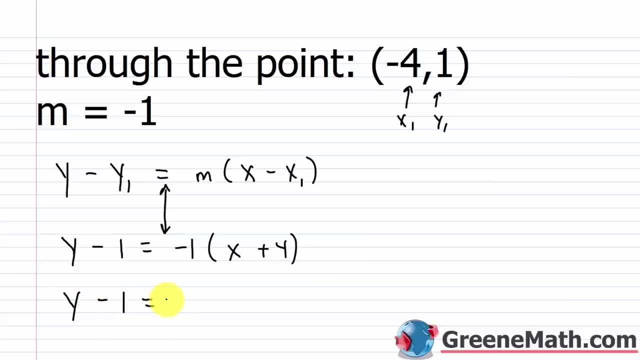 So kind of continuing here, I would have y minus 1 is equal to negative 1 times x is just negative x. 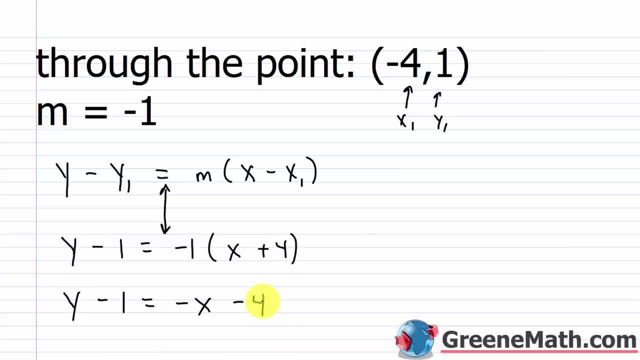 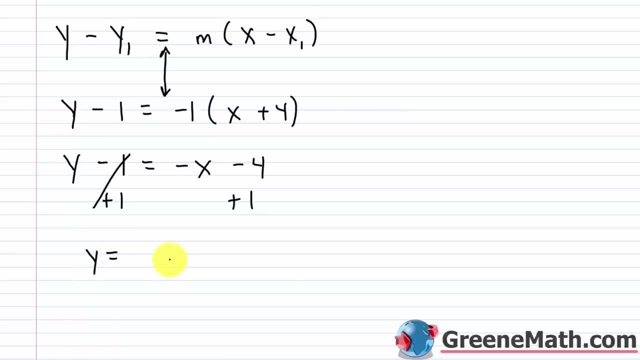 Negative 1 times 4 is just minus 4. And I would add 1 to both sides of the equation. So that would cancel. And I would have y is equal to. I'll have negative x. Negative 4 plus 1 is negative 3. So minus 3. And this is slope intercept form. 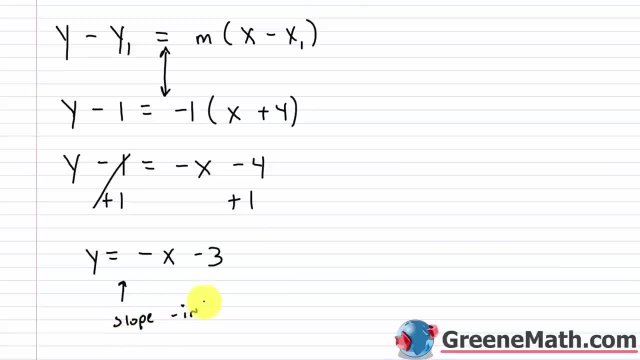 This is slope intercept form. 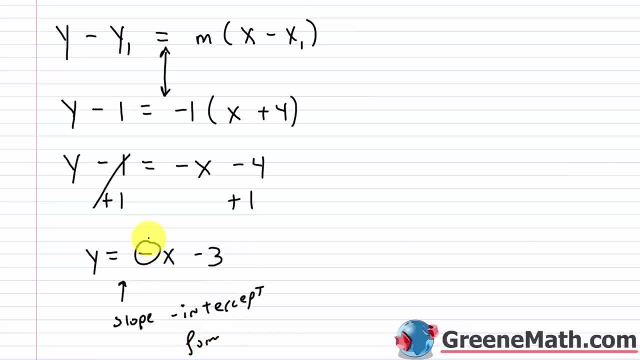 I know my slope. It's negative 1. If I have a negative out in front of x, that's the same as negative 1. 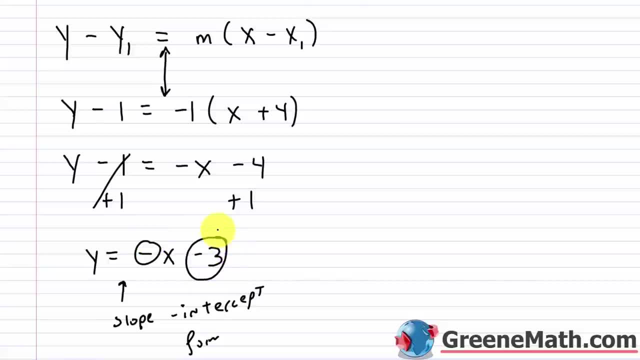 And my y intercept occurs at 0 comma negative 3. So that's slope intercept form. 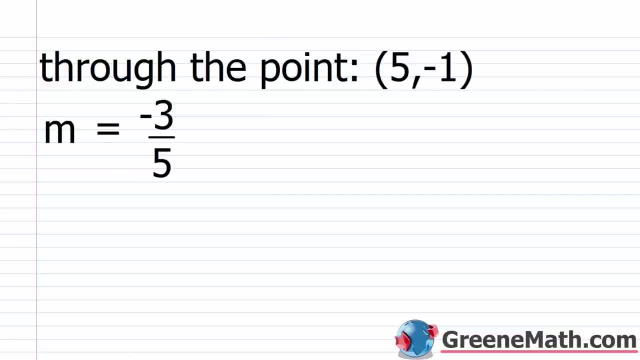 So what if we have one that's through the point 5 comma negative 1, and the slope is given to us as negative 3 fifths. So again, I would label this as x sub 1, y sub 1. And my generic point slope formula is y minus y sub 1 is equal to m times the quantity x minus x sub 1. 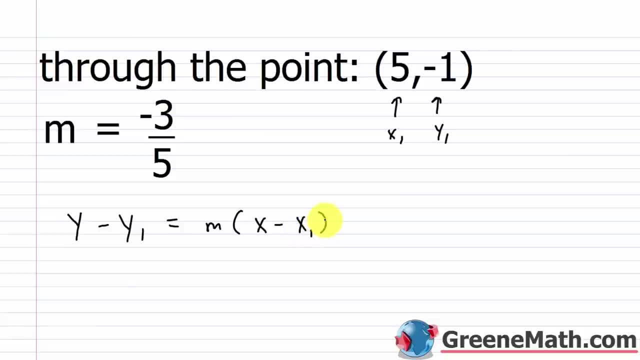 Again, especially when you first start out. You don't know this by heart. Write it out so you don't make a simple mistake. And then you plug in. It's very, very easy. So for y sub 1, I have negative 1. So I can just erase this and put minus and negative 1 is the same as plus 1. For m, I have negative 3 fifths. So negative 3 fifths. 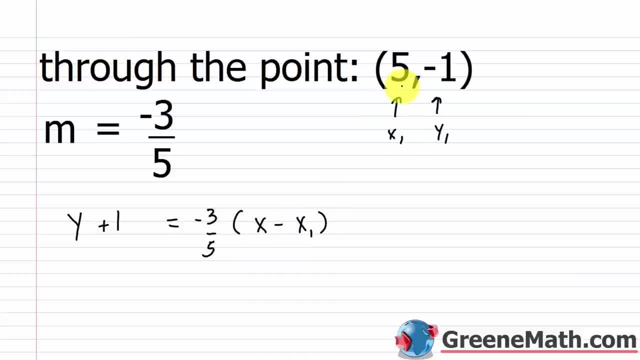 And then we have x minus x sub 1. So for x sub 1, I have 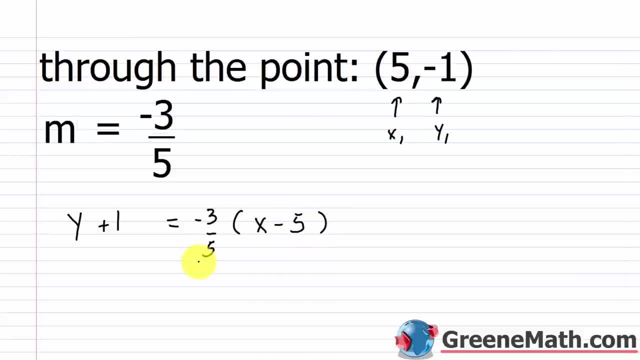 5. So this is point slope form. 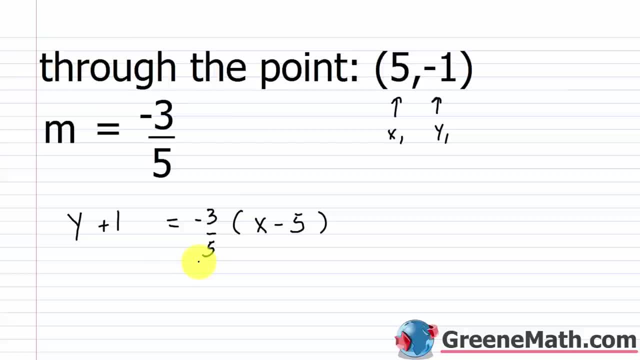 Again, if your book asked for that, you could stop there. But in most situations, they want you to solve for y and put it in slope intercept 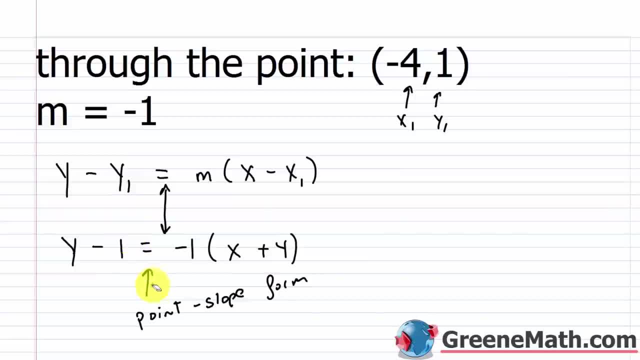 So I've done my job, But in most cases they want you to solve it for y sub 1.. So let's go ahead and do that, So kind of continuing here I would have. y minus 1 is equal to negative 1 times x is. 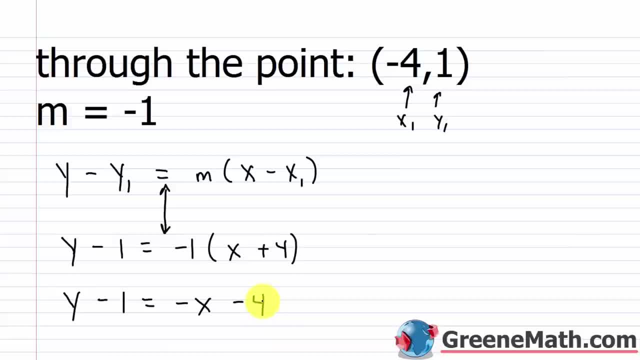 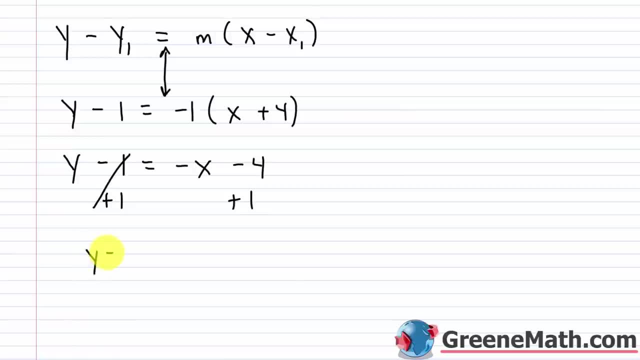 just negative x. Negative 1 times 4 is just minus 4. And I would add 1 to both sides of the equation So that would cancel And I would have y is equal to. I'll have negative x Negative. 4 plus 1 is. 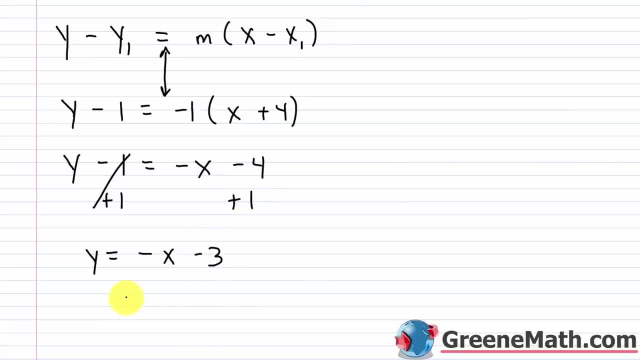 negative 3. So minus 3. And this is slope-intercept form. This is slope-intercept form. I know my slope. It's negative 1, right. If I have a negative out in front of x, that's the same as negative 1. And my y-intercept occurs at 0 comma, negative 3.. 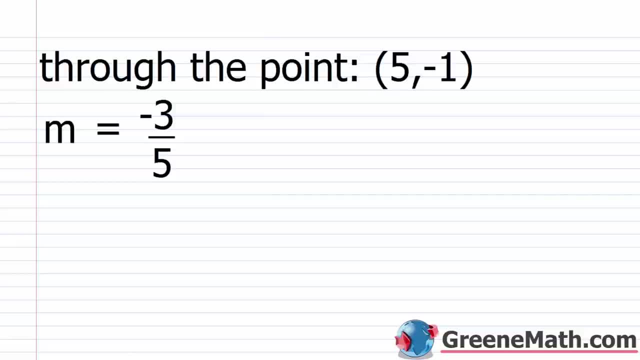 So that's slope-intercept form, All right. So what if we have one that's, through the point 5 comma, negative 1, and the slope is given to us as negative 3 fifths. So again, I would label this as x sub 1, y sub 1.. And my generic point-slope formula: 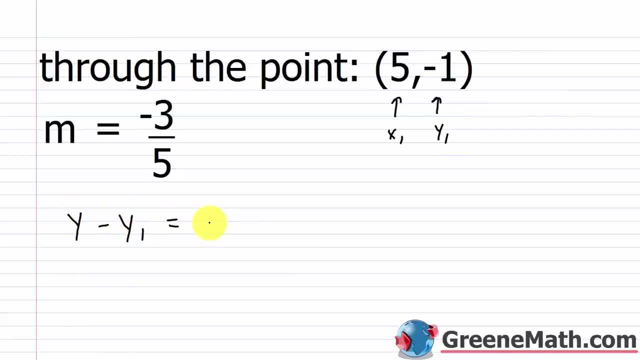 is y minus y sub 1 is equal to m times the quantity x minus x sub 1.. Again, especially when you first start out, you don't know this by heart. Write it out so you don't make a simple mistake And then you just plug in. It's very, very easy. So for y sub 1, I have negative 1.. 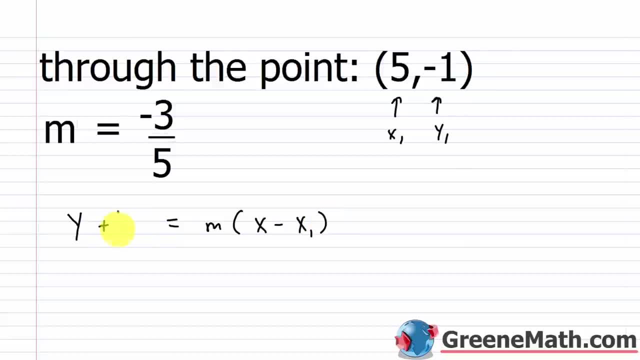 So I can just erase this and put minus a negative 1 is the same as plus 1.. For m, I have negative 3 fifths, So negative 3 fifths, And then we have x minus x sub 1.. So for x sub 1,. 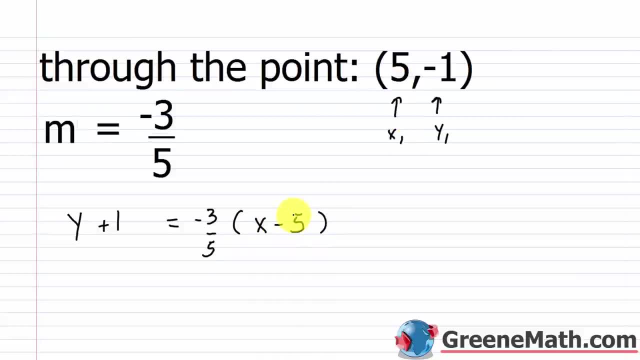 I have 5. So this is point-slope form. Again, if your book asked for that, you could stop there, But in most situations they want you to solve for y and put it in slope-intercept form. So we would continue simplifying. So y plus 1 equals negative 3 fifths times x is negative 3 fifths x. 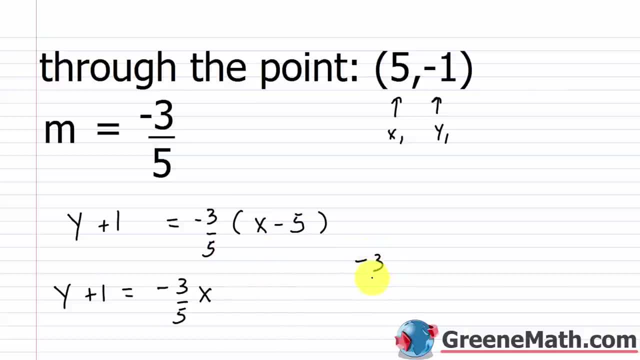 And then negative 3, fifths times negative, 5. You think about that separately over here. This would cancel with this And I'd have 1.. So basically negative 3 times negative. 1 is positive, 3. So positive 3 or plus 3 here, And so now all I have to do is subtract 1 away from each side. 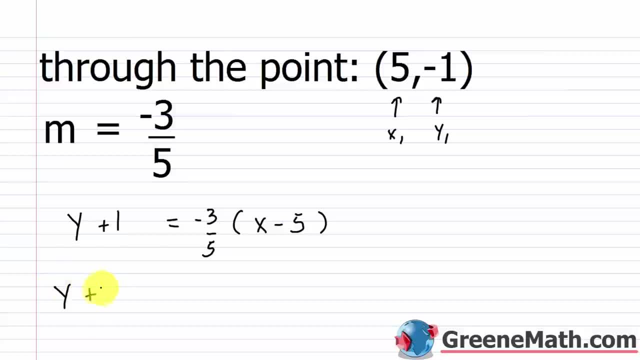 form. So we would continue simplifying. So y plus 1 equals negative 3 fifths times x is negative 3 fifths x. 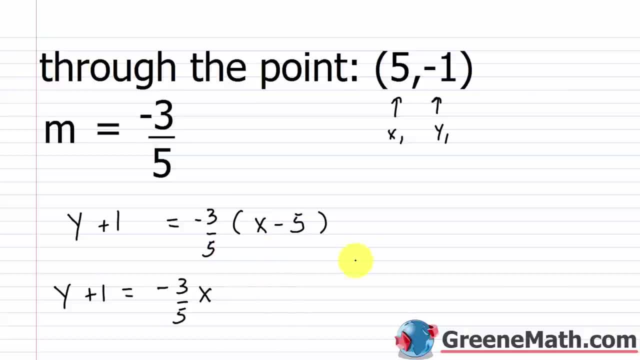 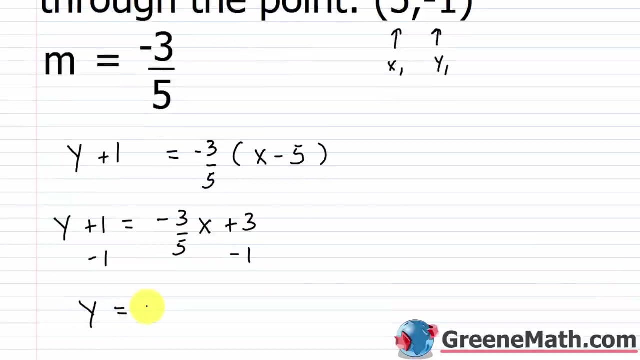 And then negative 3 fifths times negative 5. You can think about that separately over here. This would cancel with this. And I'd have 1. So basically negative 3 times negative 1 is positive 3. So positive 3 or plus 3 here. And so now all I have to do is subtract 1 away from each side so that y can be by itself. So I would have y is equal to negative 3 fifths x. 3 minus 1 is 2. So plus 2. 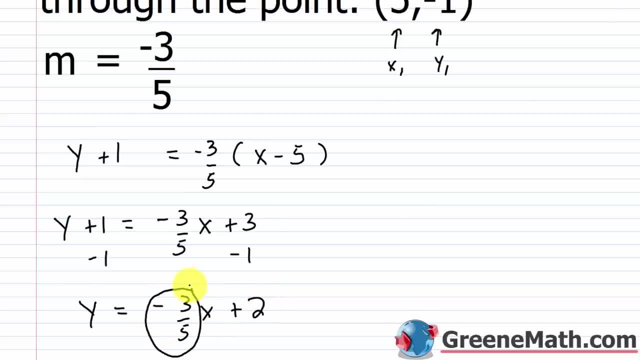 And again, this is in slope intercept form. I know that my slope is negative 3 fifths. And we were told that in the beginning. And my y intercept occurs 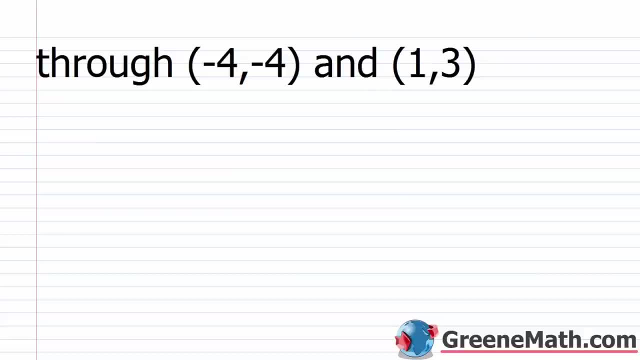 Alright, so a little bit later on in this kind of section where you're talking about equations 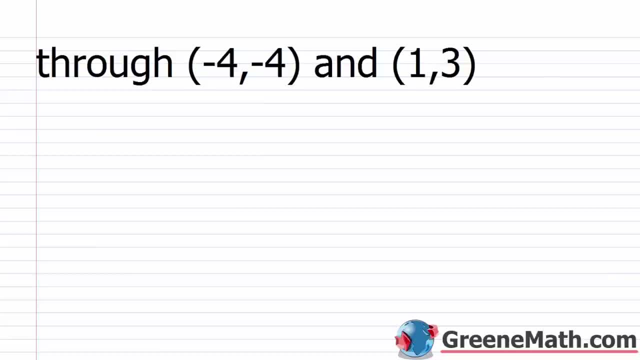 of a line, they're going to throw kind of a wrench in your plans. So you'll see this randomly and you'll be given two points and they'll say go ahead and write the equation of this line in point slope form and also in slope intercept form. 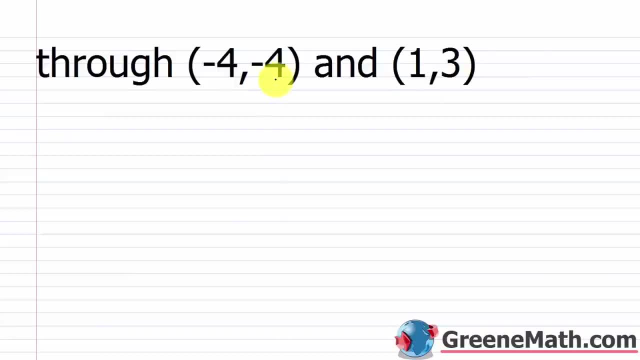 Now if I'm just given two points, how am I going to do that? Well, remember to use point slope form I need one point one point and I need the slope. So I have two points, right? I have more than I need in terms of points, but I don't know what the slope is. 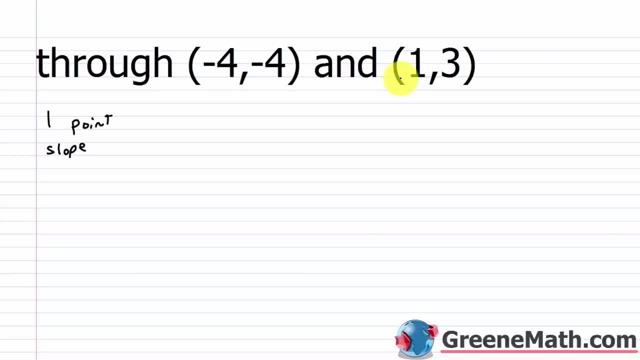 So how would you suggest we get the slope? Remember, if I have two points I can generate the slope using the slope formula. So this is something you kind of have to figure out because a lot of textbooks just leave it out. They throw the problem in there and they want you to do some critical thinking. So essentially what you're going to do is calculate your slope. So m equals y sub 2 minus y sub 1 over x sub 2 minus x sub 1. And then go back through, again any one can be x sub 2 and this could be y sub 2 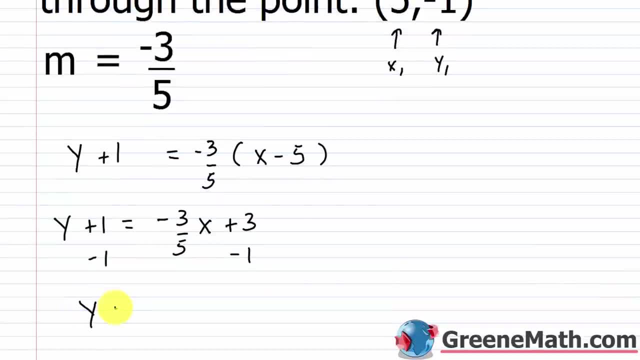 so that y can be by itself. So I would have: y is equal to negative 3 fifths x. 3 minus 1 is 2.. So plus 2.. And again, this is in slope-intercept form. I know that my slope is. 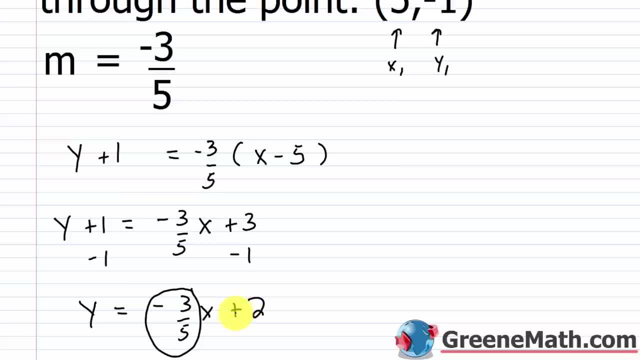 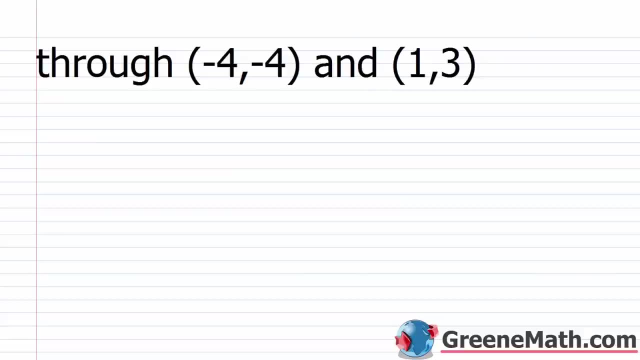 negative 3 fifths. And we were told that in the beginning, And my y-intercept occurs at 0, 2.. 0, 2.. All right, So a little bit later on, in this kind of section where you're talking about equations of a line they're going to throw. 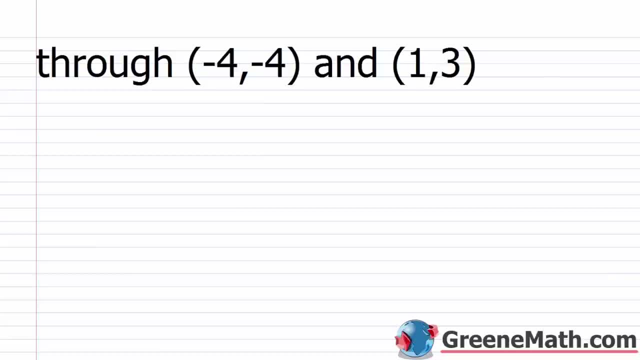 kind of a wrench in your plans. So you'll see this randomly and you'll be given two points and they'll say: go ahead and write the equation of this line in point slope form and also in slope intercept form. Now, if I'm just given two points, how am I going to do that? Well, remember to use 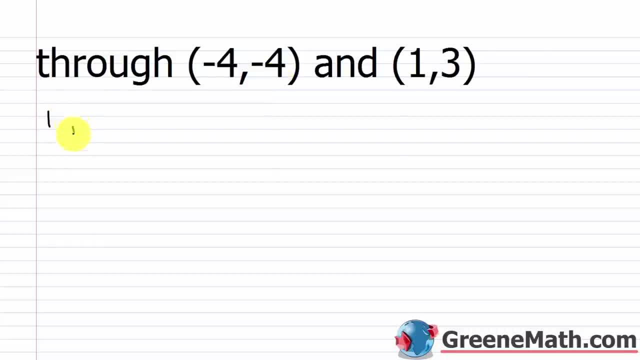 point slope form. I need one point, one point and I need the slope. So I have two points right. I have more than I need in terms of points, but I don't know what the slope is. So how would you suggest we get the slope? Remember, if I have two points, I can generate the slope using the. 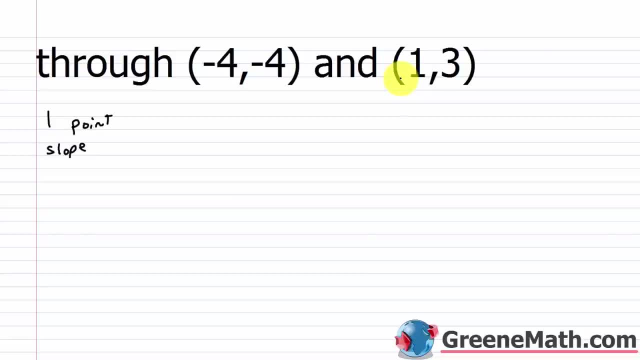 slope formula. So this is something you kind of have to figure out, because a lot of textbooks just leave it out. They throw the problem in there and they want you to do some critical thinking. So essentially, what you're going to do is calculate your slope. So 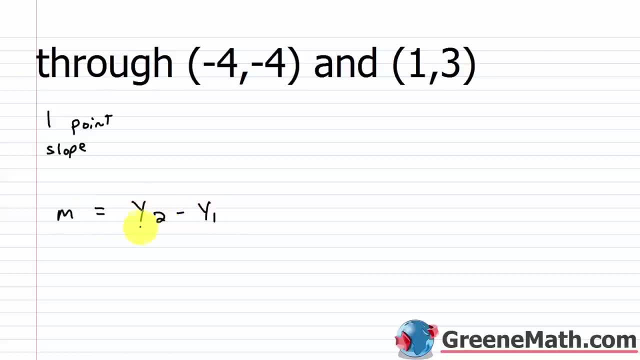 m. m equals y sub two minus y sub one, over x sub two minus x sub one, And then go back through again. any one can be x sub two, And this could be y sub two, And then this is going to be x sub. 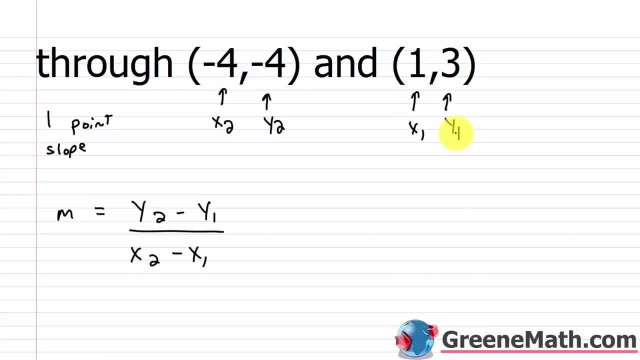 one. This will be y sub one And we just plug in. So y sub two is negative four, So negative four. And y sub one is three. X sub two is negative four also. So y sub two is negative four, So negative four. 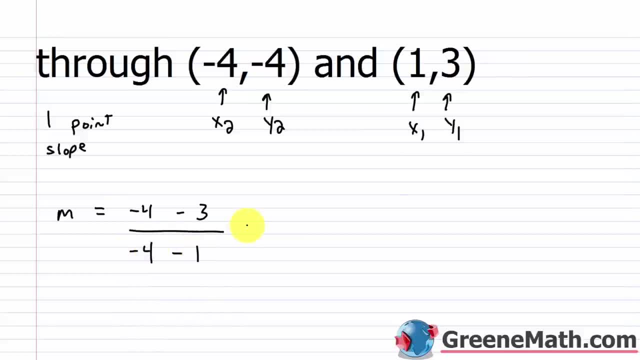 And then x sub one is one, So negative four minus three is negative seven. Negative four minus one is negative five, So negative seven over negative five is seven fifths. So I have my slope now. So m is seven fifths. So once I figured that out. 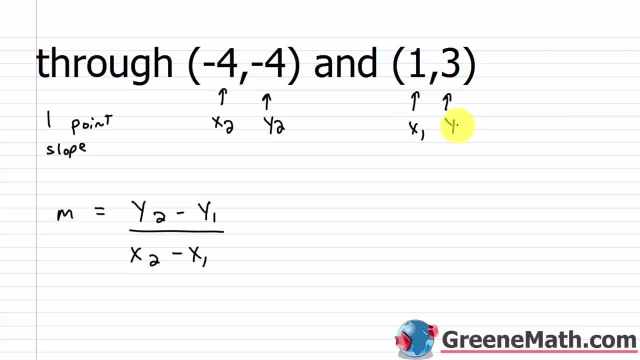 and then this is going to be x sub 1 and this will be y sub 1 and we just plug in. So y sub 2 is negative 4 so negative 4 and y sub 1 is 3 x sub 2 is negative 4 also and then x sub 1 is 1 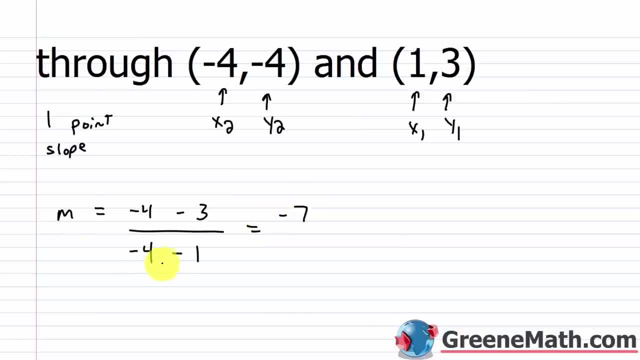 So negative 4 minus 3 is negative 7 negative 4 minus 1 is negative 5 So negative 7 over negative 5 is 7 fifths 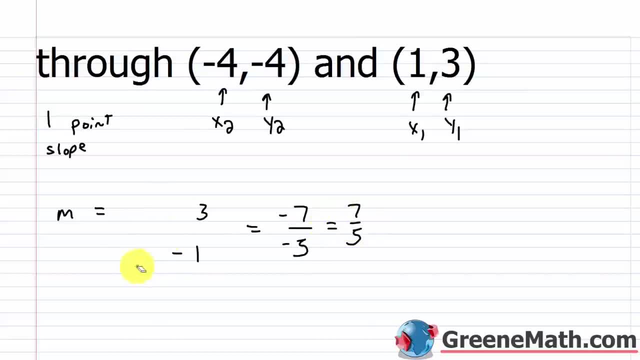 So I have my slope now So m is 7 fifths So once I've figured that out I have all the information to write an equation in point slope form. I have one point and I have a slope But some of you will get confused now because you have two points to choose from and you'll say well which point do I need to use for point slope form? Well the answer is whichever one you want. It doesn't matter. And I'm going to do it using both points just to show 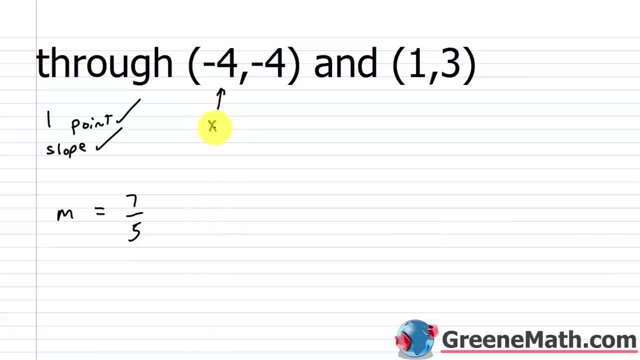 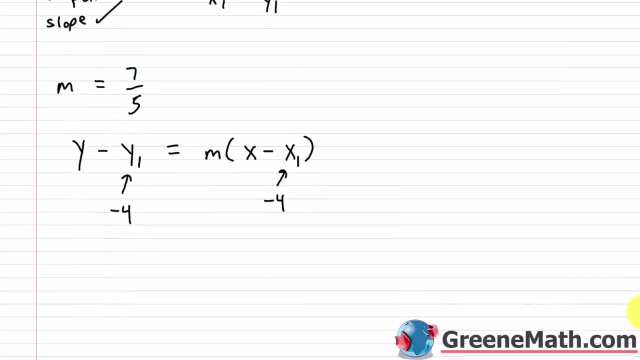 you that. So let's start out by using this one and saying this is x sub 1 y sub 1 and the point slope formula is y minus y sub 1 is equal to m times the quantity x minus x sub 1 Now I will plug in a negative 4 for y sub 1 I will plug in a negative 4 for x sub 1 So let's simplify this So we'll have y plus 4 right minus the negative 4 is plus 4 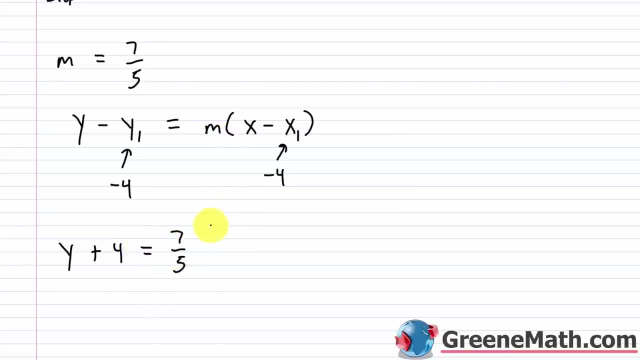 equals for m remember that's 7 fifths times the quantity x minus a negative 4 so that's plus 4 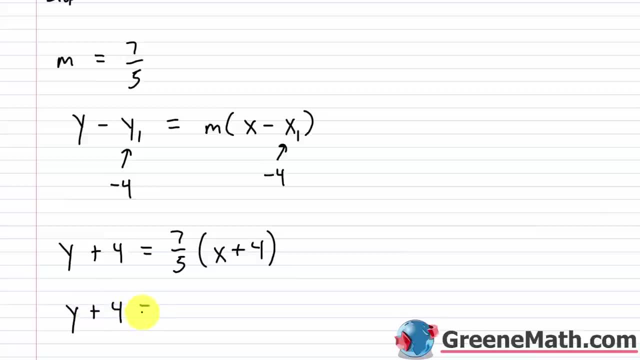 Alright so then we'd have y plus 4 is equal to 7 fifths times x plus 7 fifths times 4. 4 times 7 is 28 so this would be 28 fifths So now continuing 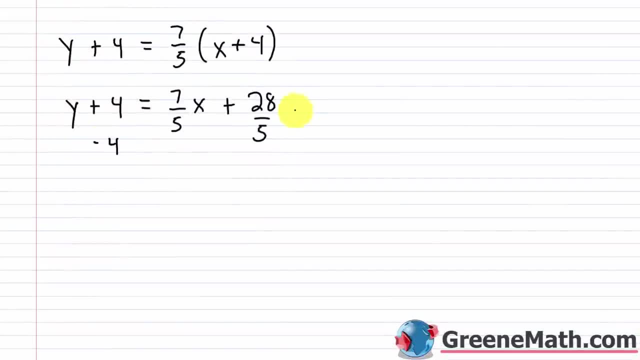 I would subtract 4 away from each side of the equation and I'm going to go ahead and write 4 as 20 over 5 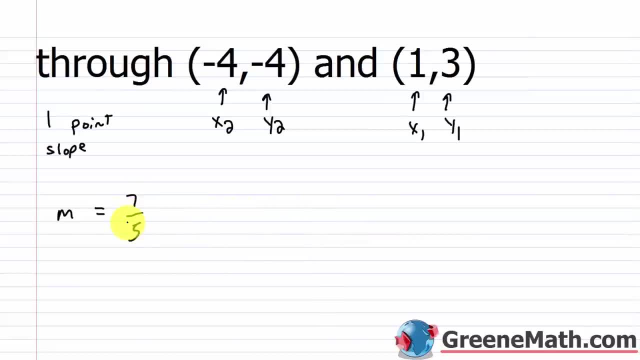 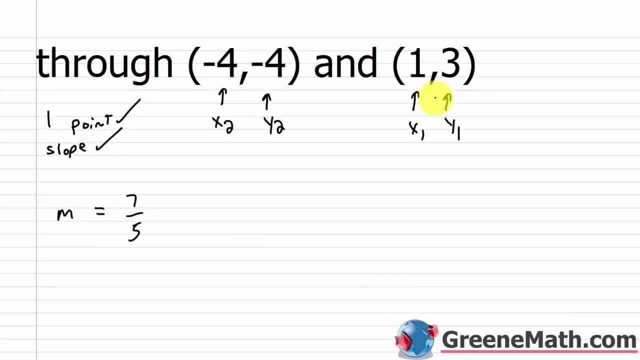 I have a slope, But some of you will get confused now because you have two points to choose from And you'll say: well, which point do I need to use for point-slope form? Well, the answer is: whichever one you want, It doesn't matter, And I'm going to do it. 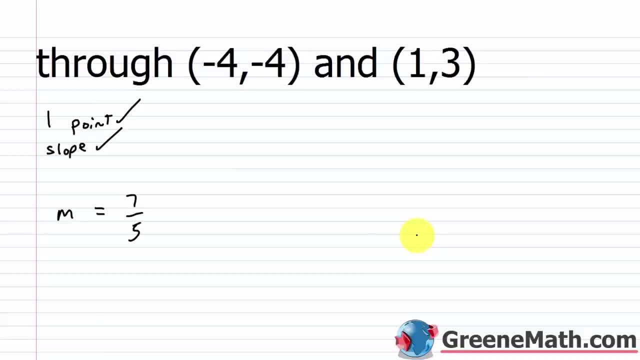 using both points just to show you that. So let's start out by using this one and saying this is x sub one, y sub one, And the point-slope formula is: y minus y sub one is equal to m times the quantity x minus x sub one. 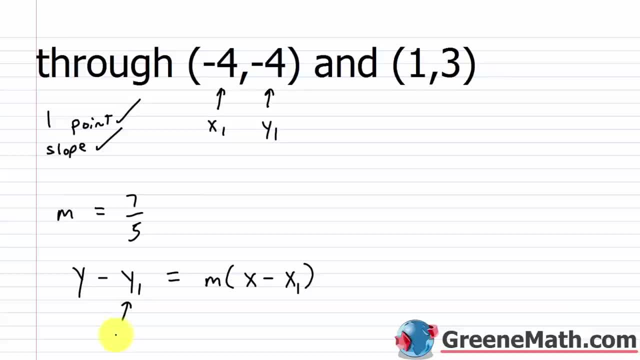 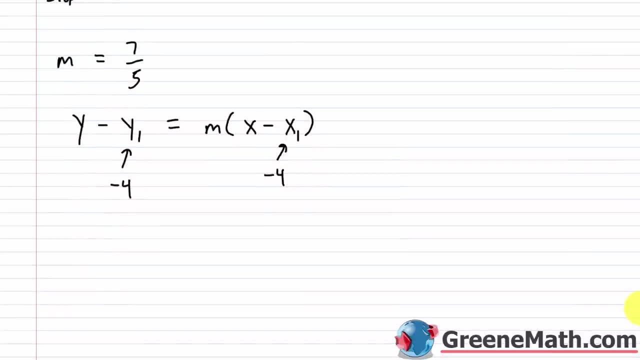 Now I will plug in a negative 4 for y sub 1.. I will plug in a negative 4 for x sub 1.. So let's simplify this. So we'll have y plus 4, right Minus. a negative 4 is plus 4.. 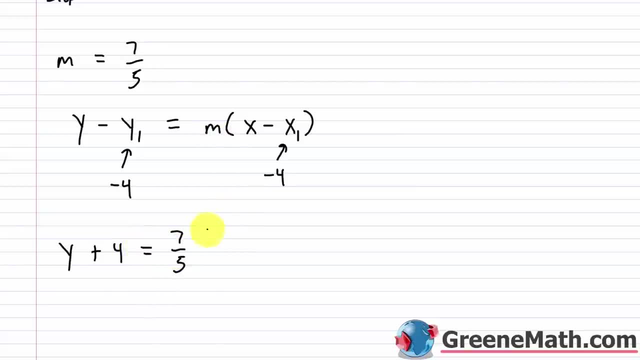 Equals for m, remember that's 7 fifths times the quantity x minus a negative 4.. So that's plus 4.. All right, So then we'd have: y plus 4 is equal to 7 fifths times x plus 7 fifths times 4.. 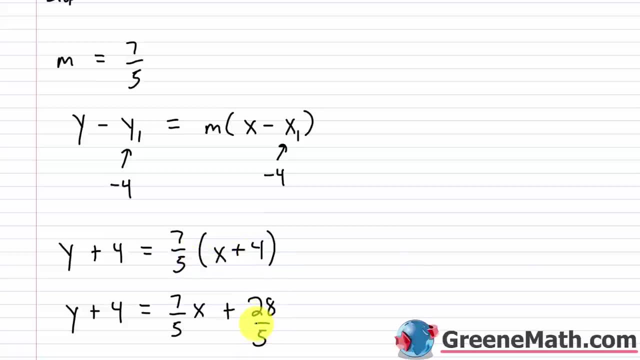 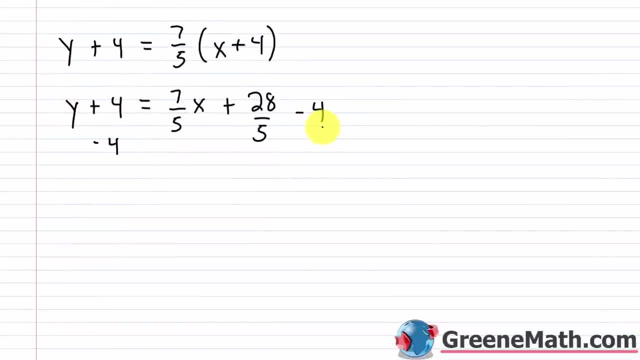 4 times 7 is 28.. So this would be 28 fifths. So now continuing, I would subtract 4 away from each side of the equation And I'm going to go ahead and write 4 as 20 over 5.. 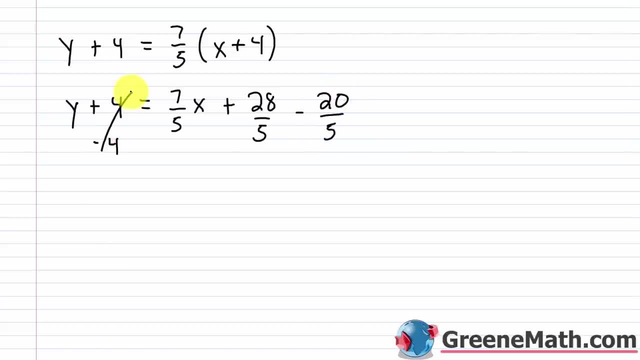 So I have a common denominator there. That's gone And I'm going to have. y is equal to 7 fifths x Plus 28 minus 20 is 8 over the denominator of 5.. So y equals 7 fifths x plus 8 fifths. 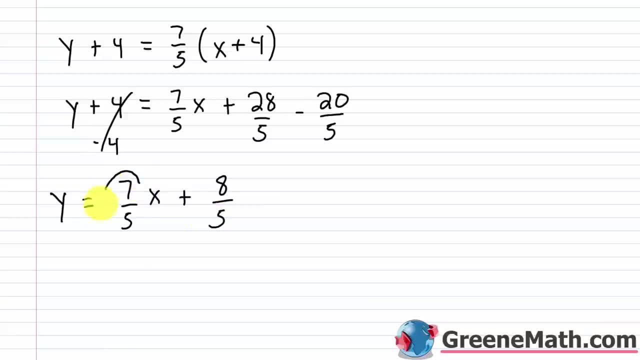 So again, this is slope-intercept form. I have my slope, which is 7 fifths. I have my y-intercept that occurs at 0 comma 8 fifths. Very, very easy. Now I want to show you using the other point, I get the same answer in the end. 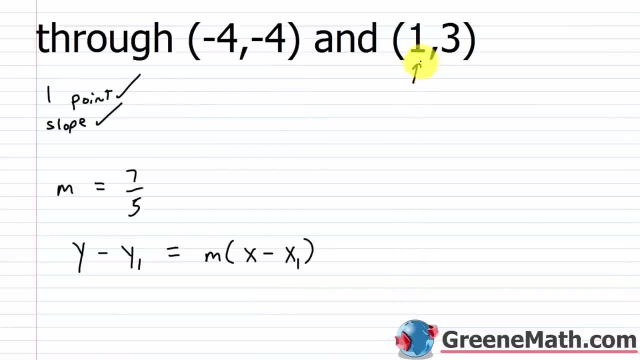 So now, let's say I had chosen to use this as my point. So this is x, So I'm going to have y sub 1, y sub 1.. So I'm just plugging in. So for y sub 1, I'm plugging in a 3.. 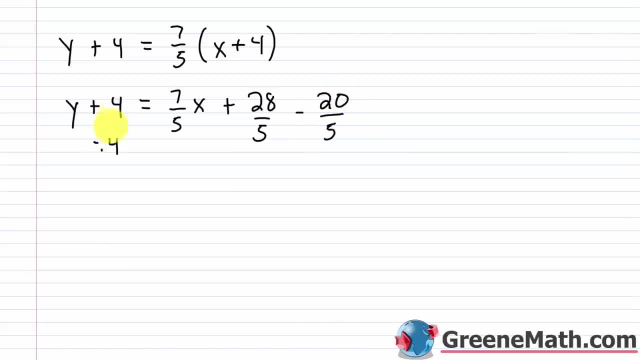 So I have a common denominator there that's gone and I'm going to have y is equal to 7 fifths x plus 28 minus 20 is 8 over the denominator of 5 So y equals 7 fifths x plus 8 fifths So again this is slope intercept form I have my slope which is 7 fifths I have my y intercept that occurs at 0 comma 8 fifths Very very easy Now I want to show you 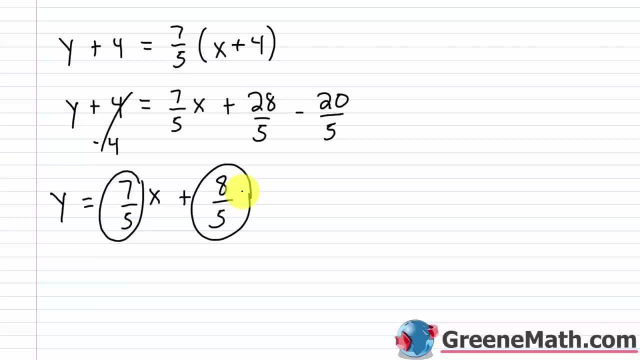 using the other point I get the same answer 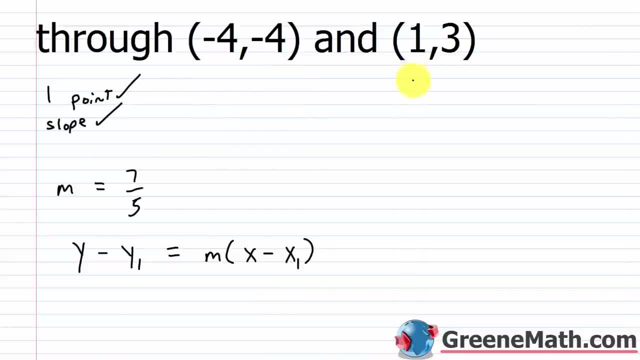 in the end. So now let's say I had chosen to use this as my point So this is x sub 1 y sub 1 so I'm just plugging in So for y sub 1 I'm plugging in a 3 For x sub 1 I'm plugging in a 1 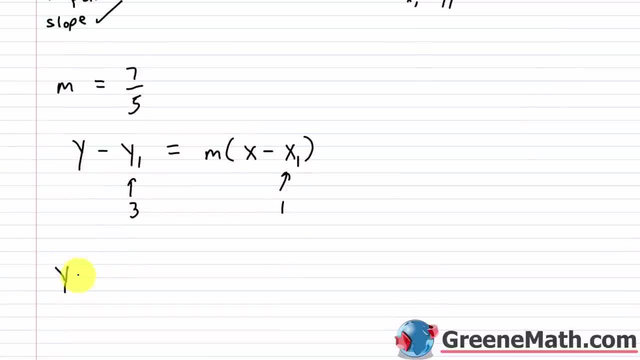 So let's crank this out So I'd have y minus y sub 1 is 3 equals m which we know is 7 fifths times the quantity x minus 1 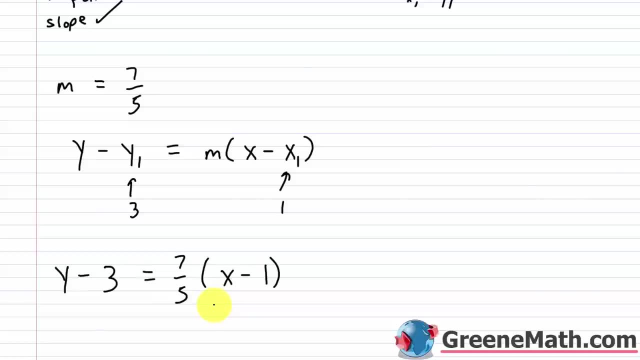 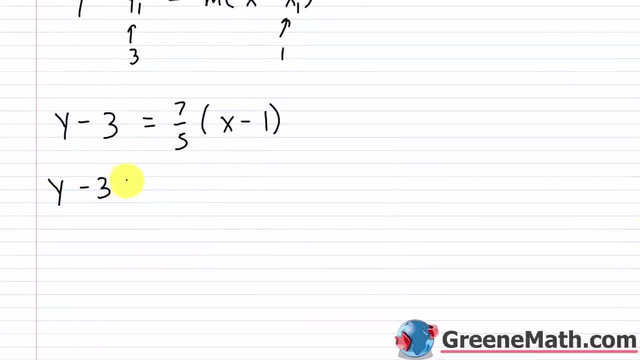 So at this point when we have it in point form it looks a little different You might say oh well that's not the same But when you solve it for y you're going to get the same thing So you'd have y minus 3 is equal to 7 fifths times x is just 7 fifths x minus 7 fifths times 1 is just 7 fifths So I would add 3 to both sides of the equation I'm going to go ahead and write 3 as 15 over 5 So I have a common denominator so that's gone y is equal to 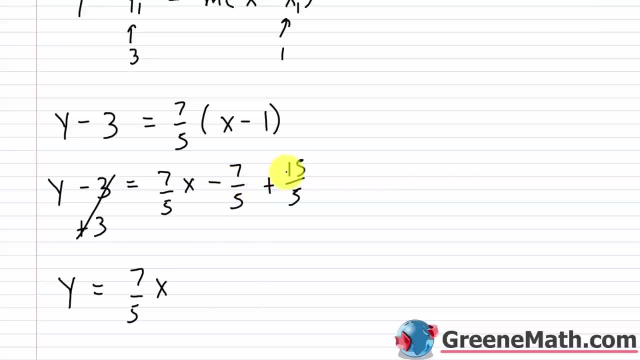 7 fifths x So we have negative 7 plus 15 What is that? That's 8 So plus 8 over that common denominator of 5 So we get the exact same thing y equals 7 fifths x plus 8 fifths 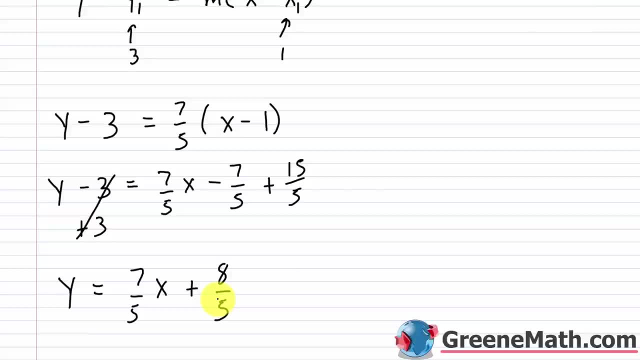 So that is using a different point So as long as that point is on that line you're good to go You can use whatever point you'd like 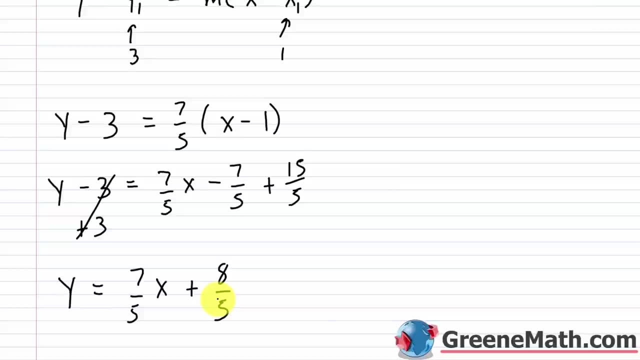 as long as you know the slope So if you have one point on the line and the slope you're going to use point slope formula 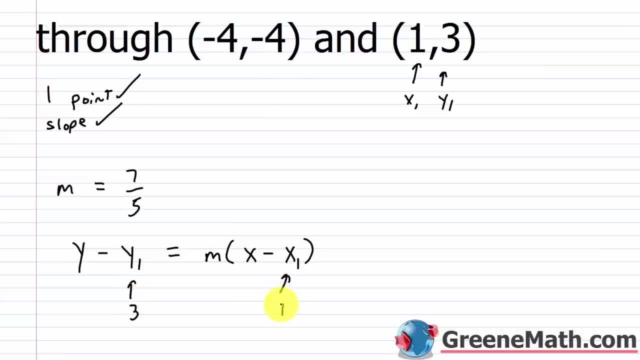 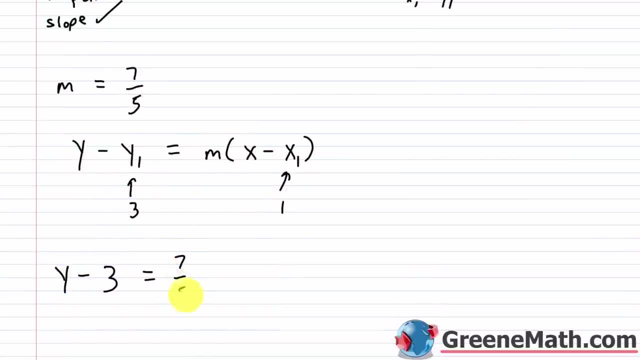 For x sub 1, I'm plugging in a 1. So let's crank this out. So I'd have: y minus y sub 1 is 3, equals m, which we know is 7 fifths times the quantity x minus 1.. 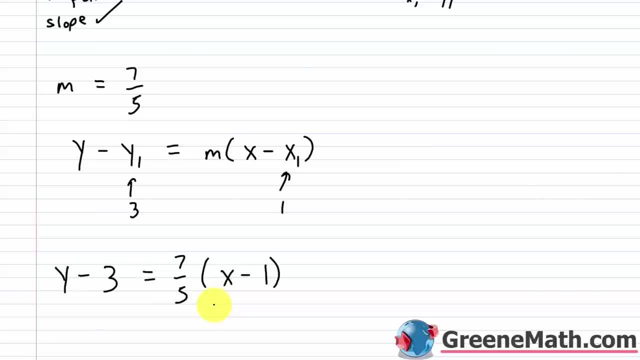 So at this point, when we have it in point-slope form, it looks a little different. You might say, oh well, that's not the same, But when you solve it for y, you're going to get the same thing. 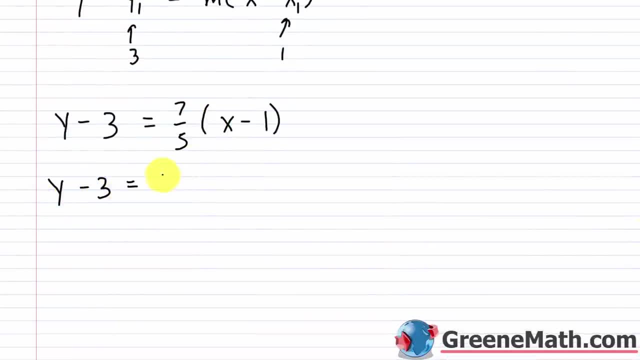 So you'd have: y minus 3 is equal to 7 fifths times x is just 7 fifths. x minus 7 fifths times 1 is just 7 fifths. So I'm going to add 3 to both sides of the equation. 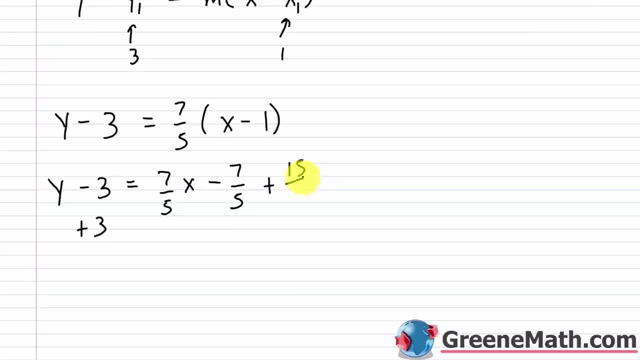 I'm going to go ahead and write 3 as 15 over 5.. So I have a common denominator. So that's gone. y is equal to 7 fifths x, So we have negative 7 plus 15.. What is that? 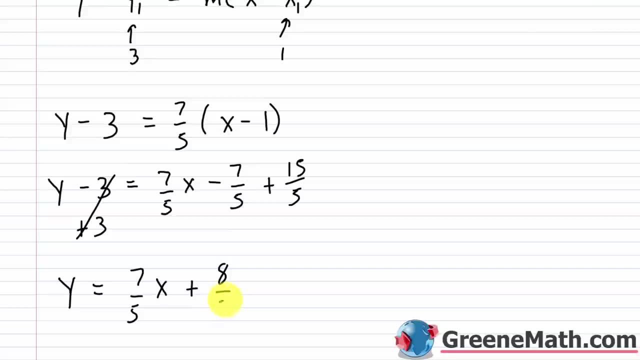 That's 8, right. So plus 8.. Over that common denominator of 5.. So we get the exact same thing. y equals 7 fifths x plus 8 fifths. So that is using a different point, right. 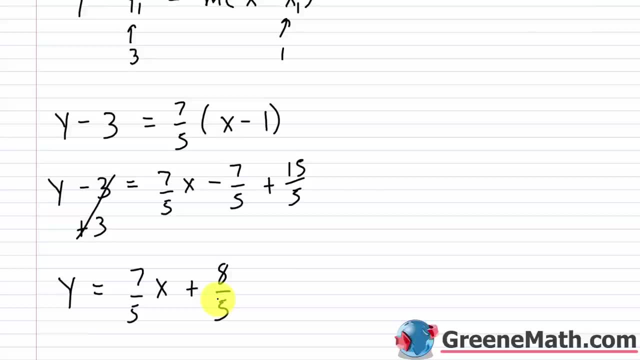 So as long as that point is on that line, you're good to go. You can use whatever point you'd like, as long as you know the slope. So if you have one point on the line and the slope, you're going to use point-slope formula. 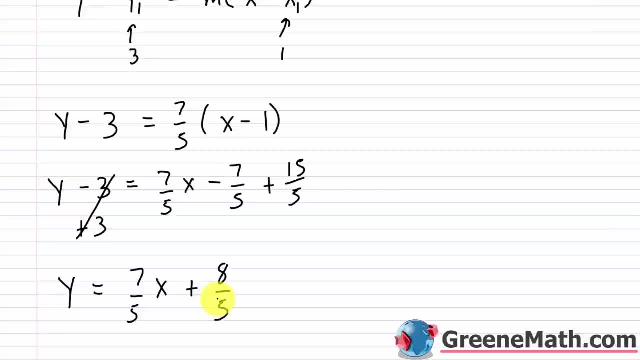 If you have two points and you're not given a slope, you're going to use point-slope formula. Just in that particular case, you got to do a little extra work, right? You got to take the two points, generate a slope. okay, using the slope formula. 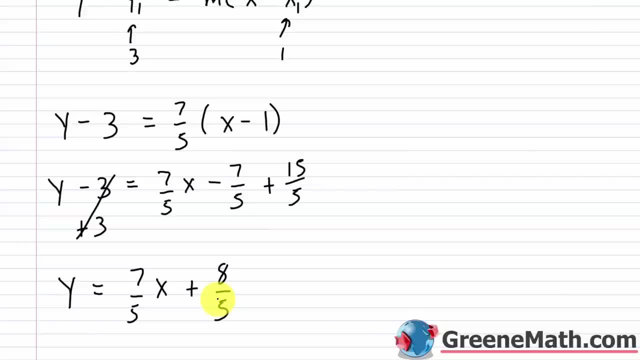 Then go back and plug in using one of the points. It doesn't matter which one. So go back and plug into the point-slope formula that you have, And then you can solve it for y and get it in slope-intercept form. 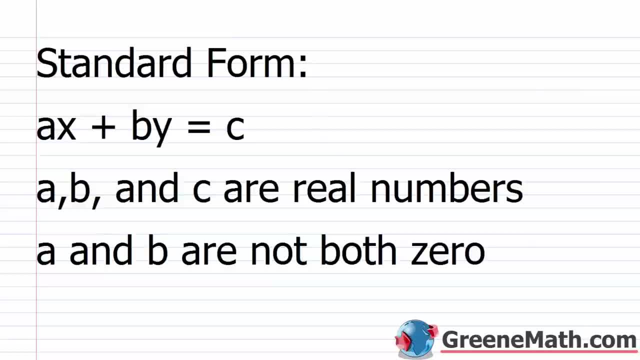 All right. So, lastly, we want to discuss something known as standard form. So the definition for standard form- I'm going to tell you this right off the bat- is going to vary between textbooks. So I'm going to give you a generic definition and then I'm going to give you the one that 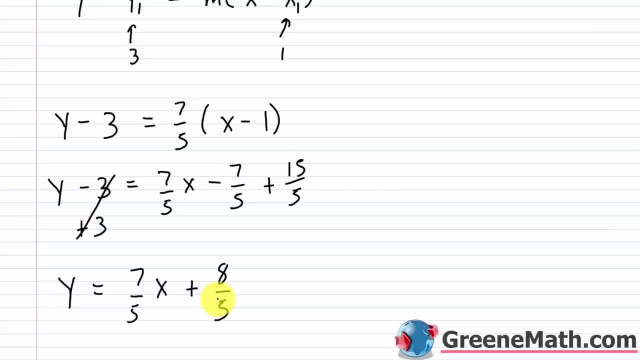 If you have two points and you're not given a slope you're going to use point slope formula Just in that particular case you've got to do a little extra work You've got to take the two points generate a slope using the slope formula then go back and plug in using one of the points It doesn't matter which one So go back and plug into the point slope formula that you have and you can solve it for y and get it in slope intercept form Alright so lastly we want to discuss 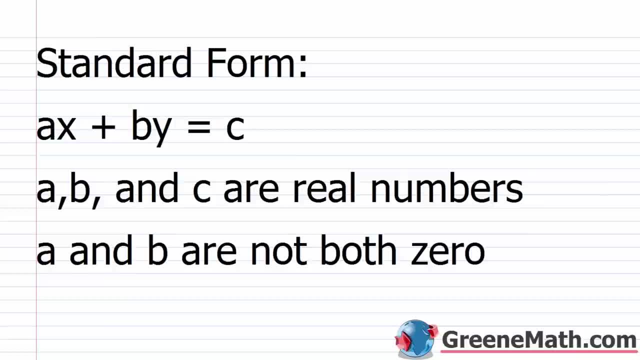 standard form So the definition for standard form I'm going to tell you this right off the bat is going to vary between textbooks So I'm going to give you a generic definition and then I'm going to give you the one that you're probably going to get when you're in high school So for standard form kind of starting out I would say in college algebra you'd say ax plus by equals c where ab and c are real numbers and a and b are not both zeros So a, b, and c can be anything you want They can be negative, they can be fractions 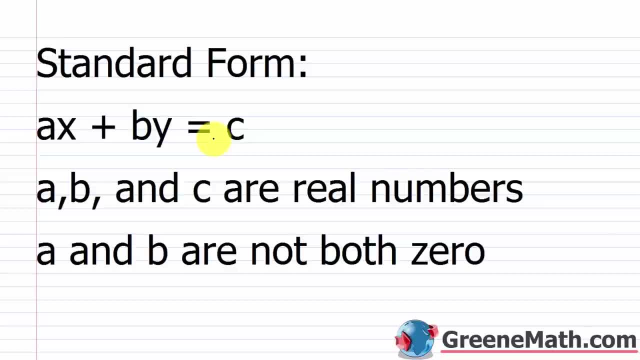 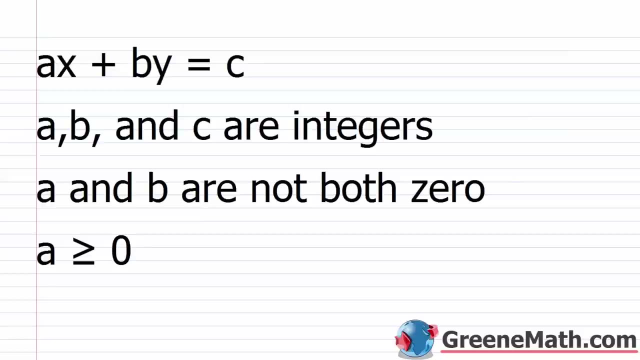 anything you want, doesn't matter Now there's a stricter version of this which you're probably going to be yelling at the screen going that's not what my teacher said It's got to be interesting So let me show you that one So the stricter version, the one that you generally learn in an algebra one or algebra two class in high school will be this ax plus by equals c where a, b, and c are integers a and b are not both zeros and they also want a to be zero or positive It's greater than or equal to zero 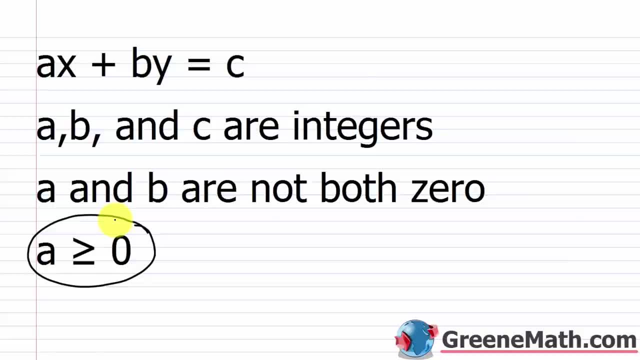 as another condition for a So with this definition you generally have a little bit more work to do 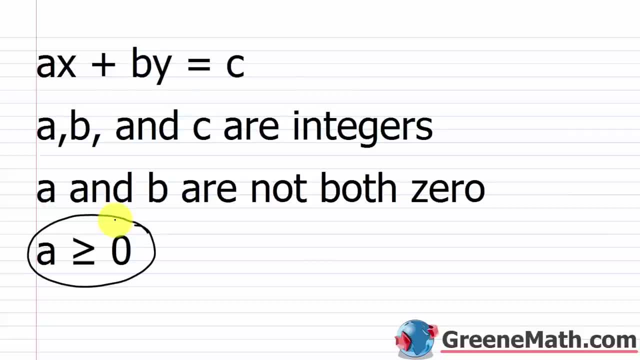 but it's all about manipulating the equation You can kind of do whatever you need to do to fulfill this definition So let's look at some quick examples here 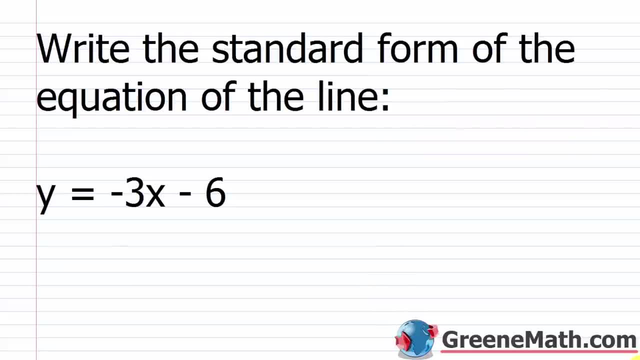 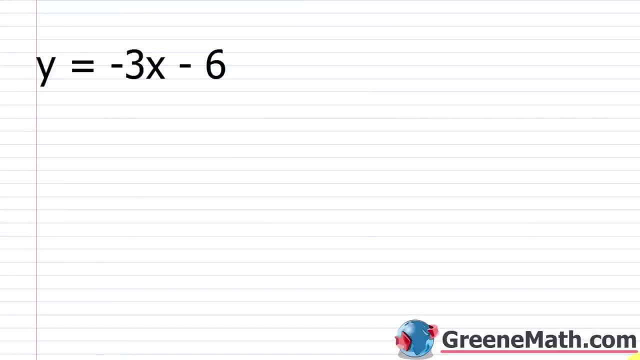 So again, write the standard form of the equation on the line We're going to use that stricter definition here because most of you are in high school and you kind of need to know how to manipulate the equation If you're watching this and you're in a higher level mathematics class and it doesn't matter 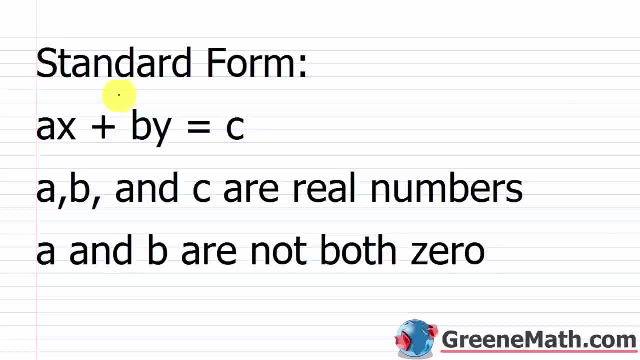 you're probably going to get when you're in high school. So for standard form, kind of starting out, I would say in college algebra you'd say ax plus by equals c, where a, b and c are real numbers and a and b are not both zeros. 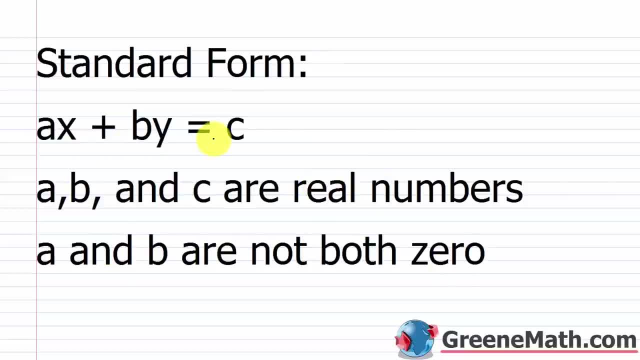 So a, b and c can be anything you want. They can be negative, They can be fractions, They can be anything you want, It doesn't matter. Now there's a stricter version of this which you're probably going to like. 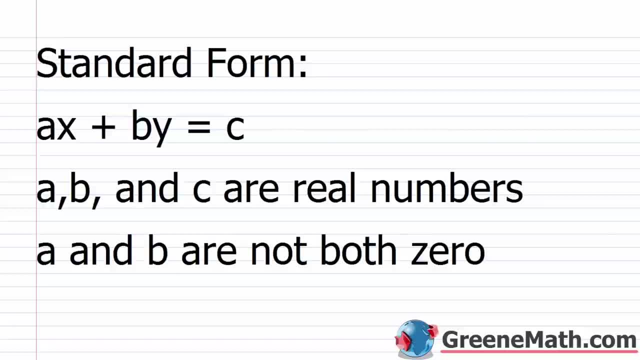 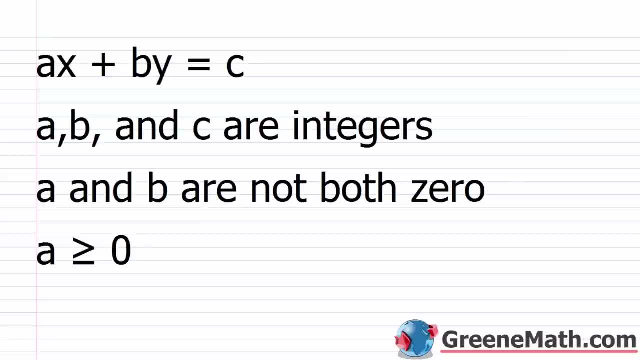 You're probably going to be yelling at the screen going: that's not what my teacher said. No, It's got to be interesting. So let me show you that one. So the stricter version, the one that you generally learn in an algebra one, or algebra. 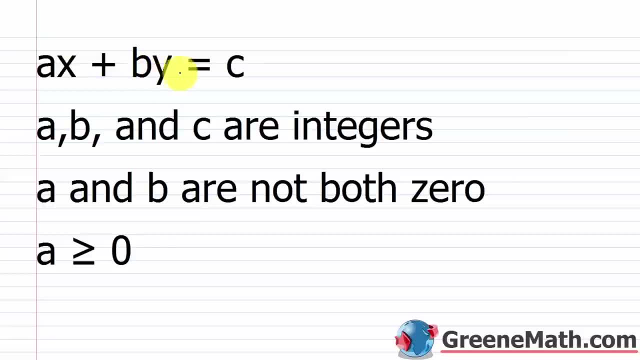 two class in high school will be this: Ax plus by equals c, where a, b and c are integers. a and b are not both zero and they also want a to be zero or positive right. It's greater than or equal to zero as another condition for a. 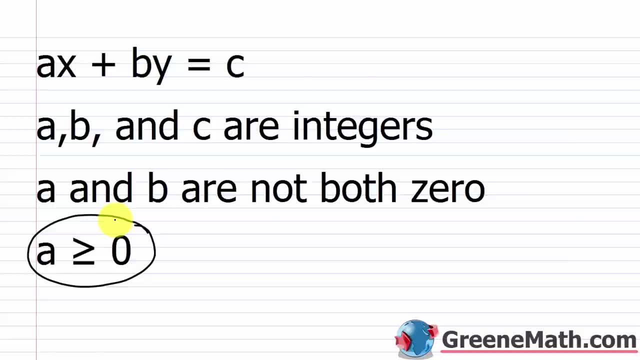 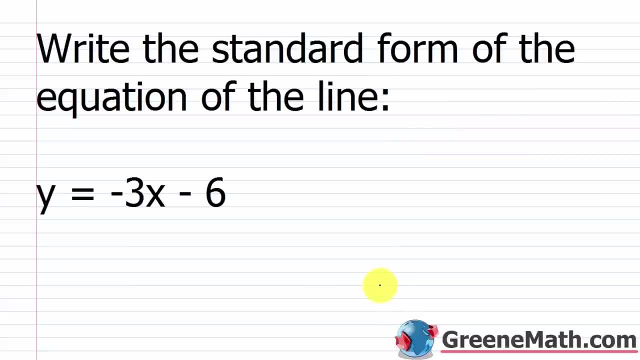 So with this definition Now, you generally have a little bit more work to do, but it's all about manipulating the equation. You can kind of do whatever you need to do to fulfill this definition. So let's look at some quick examples here. 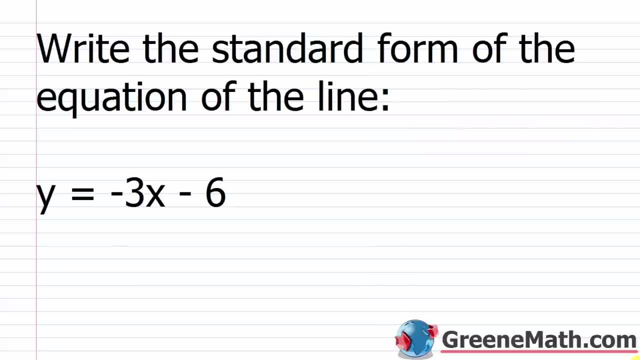 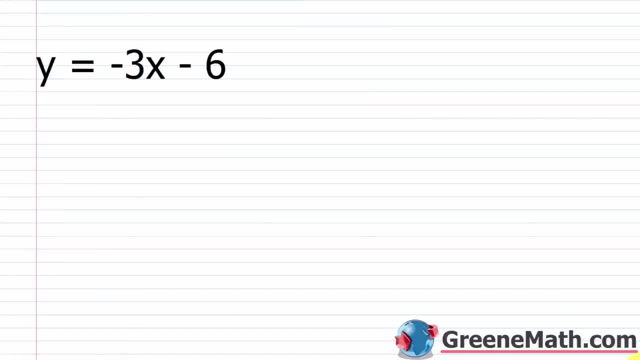 So again, write the standard form of the equation, of the line. We're going to use that stricter definition here because most of you are in high school and you kind of need to know how to manipulate the equation. If you're watching this and you're in a higher level mathematics class and it doesn't matter. 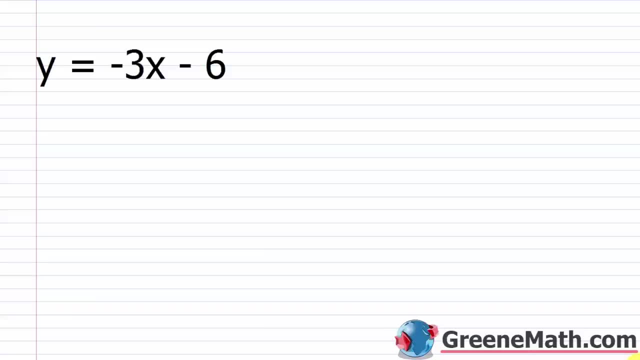 then you kind of just get to practice anyway on how to manipulate an equation. So again, we want a to be greater than zero. We want a to be greater than or equal to zero- That's the coefficient of x- And we want a, b and c to be integers. 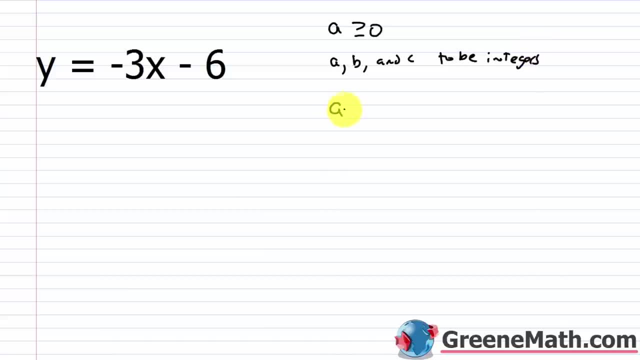 We know that a and b can't both be zero, and so it looks like this: ax plus by equals c. So how would I get y equals negative, 3x minus 6 to look like that? Well, I'd start by adding 3x to both sides of the equation. 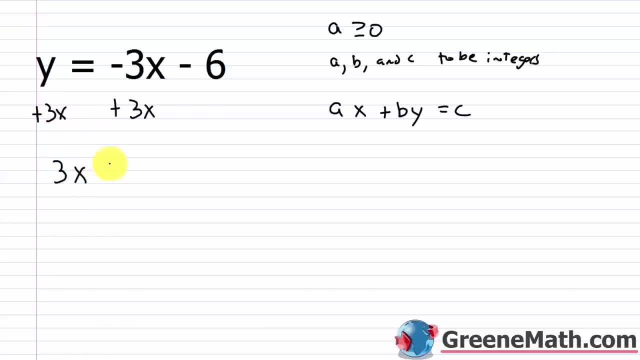 And I'd have: 3x plus y equals c, That's the coefficient of x Plus y is equal to negative 6.. So at this point I'm actually done. I've satisfied all the requirements. a and b are not both zero. 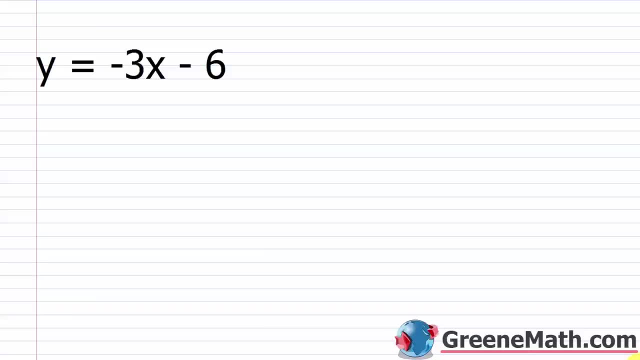 you kind of just get the practice anyway on how to manipulate an equation So again, we want a to be greater than or equal to zero that's the coefficient of x and we want a, b, and c to be integers 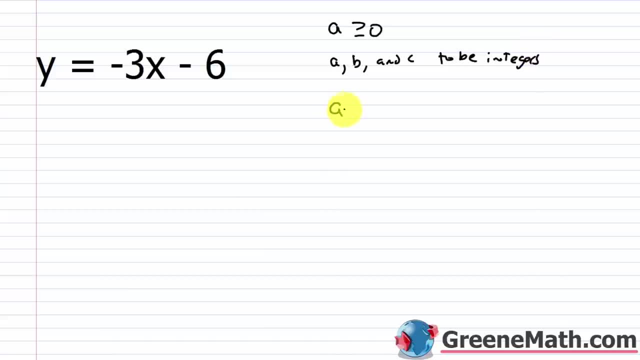 We know that a and b can't both be zero and so it looks like this ax plus by equals c 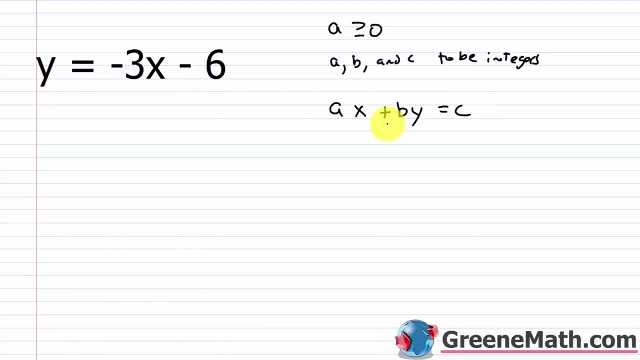 So how would I get y equals negative 3x minus 6 to look like that Well I'd start by adding 3x to both sides of the equation and I'd have 3x plus y is equal to negative 6 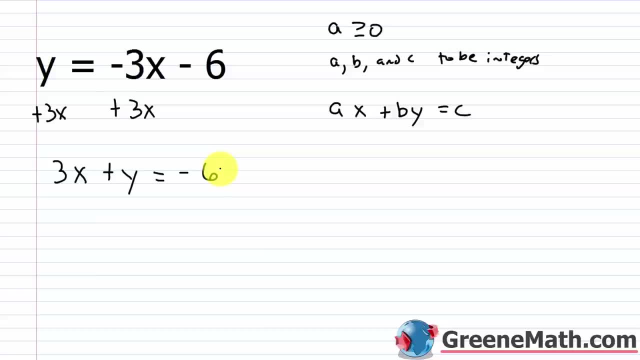 So at this point I'm actually done I've satisfied all the requirements a and b are not both zero none of them are zero a, b, and c are all integers 3 is an integer this you can think of as 1 so that's an integer and negative 6 is an integer and a is greater than or equal to zero very very easy all I had to do was add 3x to both sides of the equation and that's kind of an easier example 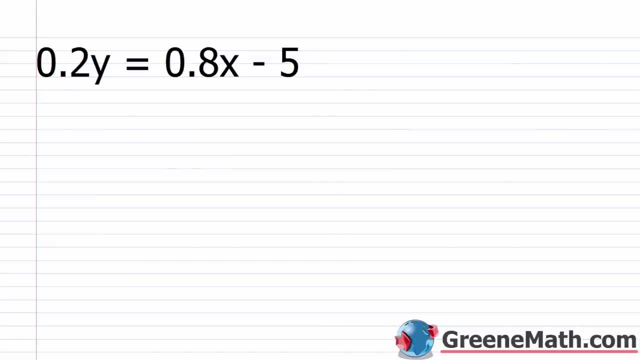 What if I got something like this 0.2y equals 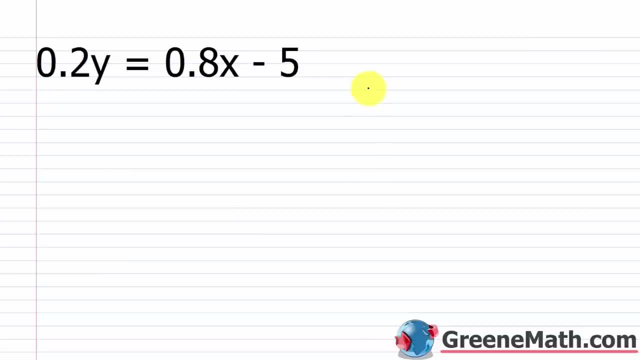 0.8x minus 5 Again, the format I want is ax plus by equals c 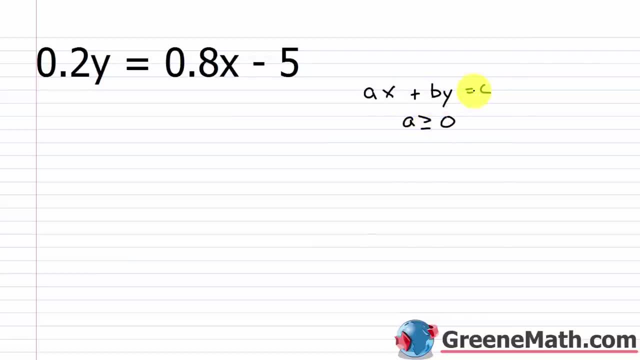 a is greater than or equal to zero a, b, and c are all integers 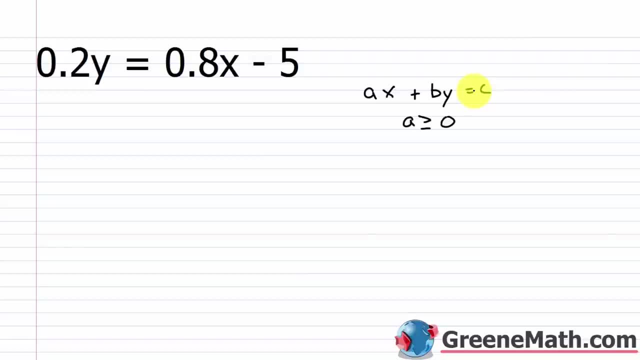 and a and b are not both zero So again, the first thing 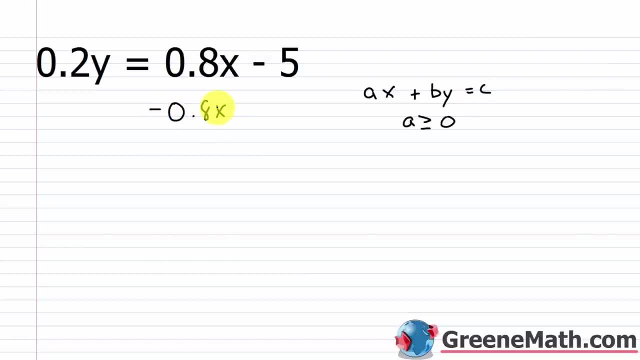 I'm going to do is subtract 0.8x from both sides of the equation So I'd have negative 0.8x and then 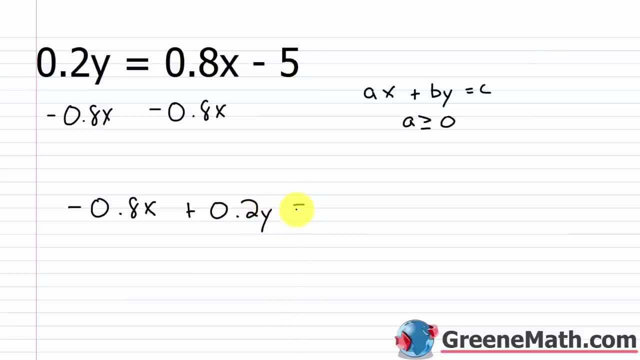 plus 0.2y is equal to negative 5 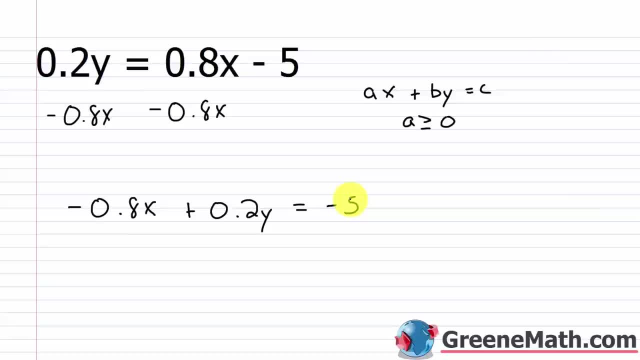 Now, I have two problems here I have the problem that this is negative this is negative and I have the problem that it's a decimal 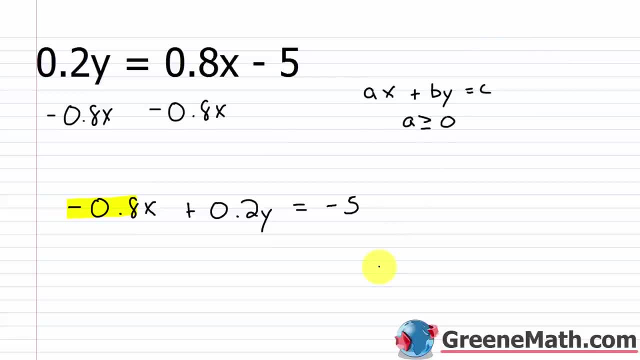 So I can fix both of them relatively easily To convert this from a decimal to a whole number or to an integer I would need to multiply by the appropriate power of 10 So in each case we have one decimal place 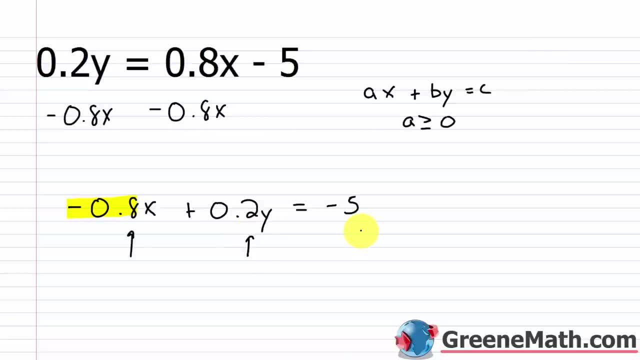 So all I would have to do is multiply both sides of the equation by 10 Very very easy So if I do that 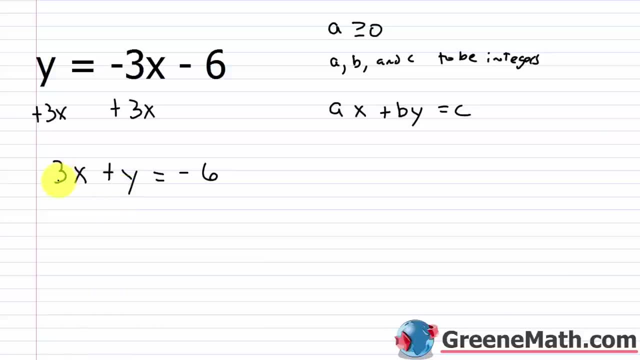 None of them are zero. a, b and c are all integers. 3 is an integer. This you can think of as 1.. So that's an integer And negative. 6 is an integer And a is greater than or equal to zero. 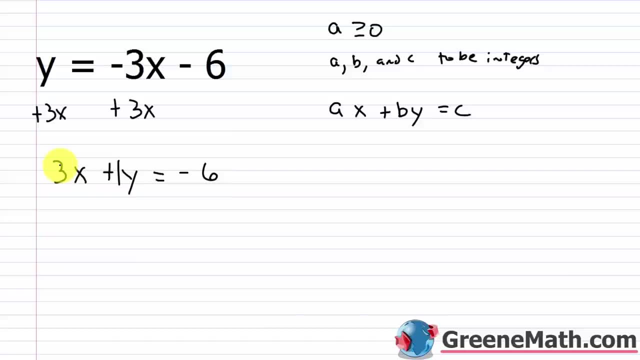 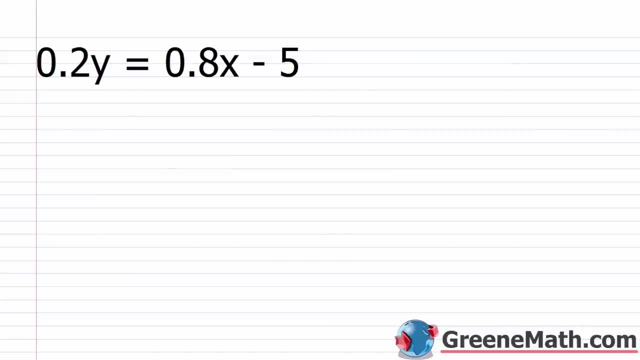 a is the coefficient on x. So we've satisfied our requirement very, very easy. All I had to do was add 3x to both sides of the equation, And that's kind of an easier example. What if I got something like this: 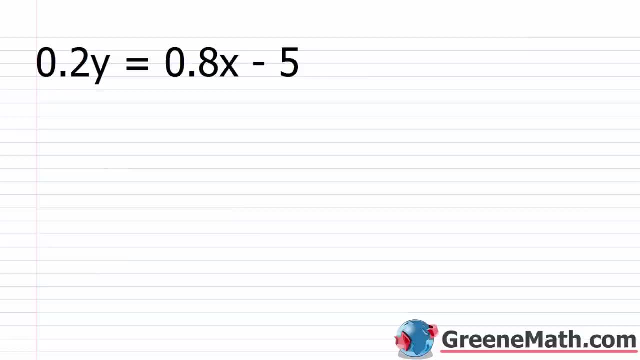 0.2y equals 0.8x minus 5.. Again, the format I want is ax plus by equals c. a is greater than or equal to zero. a, b and c are all integers, And a and b are not both zero. 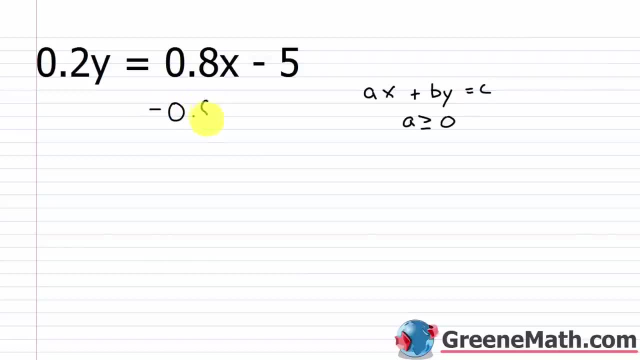 So, again, the first thing I'm going to do is subtract 0.8x from both sides of the equation, So I'd have negative 0.8x. 0.8x and then plus 0.2y is equal to negative 5.. 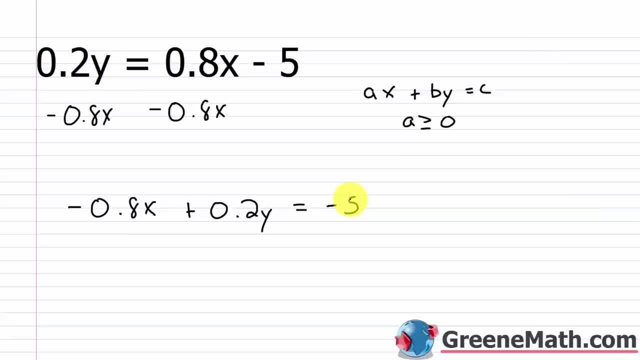 Now I have two problems here. I have the problem that this is negative. This is negative, And I have the problem that it's a decimal. So I can fix both of them relatively easily To convert this from a decimal to a whole number. 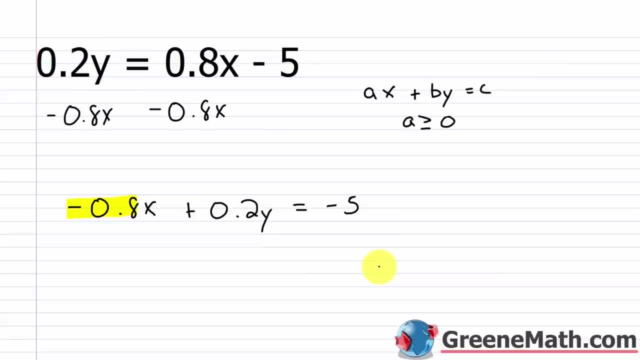 or to an integer. I would need to multiply by the appropriate power of 10.. So in each case we have one decimal place. So all I would have to do is multiply both sides of the equation by 10.. Very, very easy. 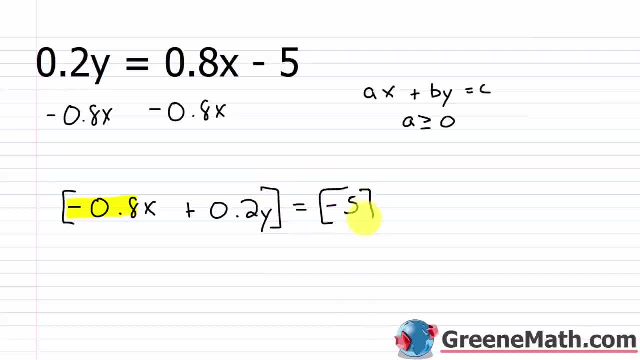 So if I do that, so 10 times negative 0.8x. Essentially, I'm just moving this one place to the right, the decimal point, So this would end up being negative 8x, Then plus 10 times 0.2y. 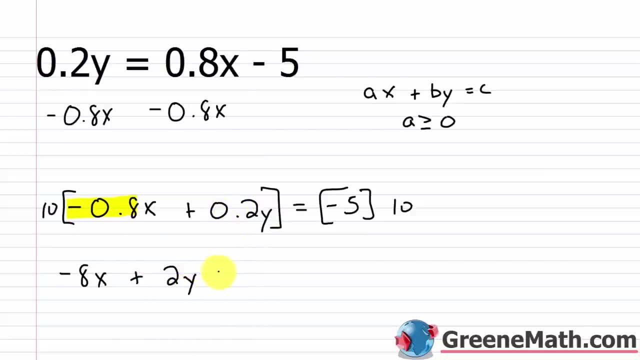 Again. I'm just moving this one place to the right. So this would be 2y. This equals 10 times negative. 5 is negative 50.. So I've solved the part where I want integers, but a is not greater than or equal to 0.. 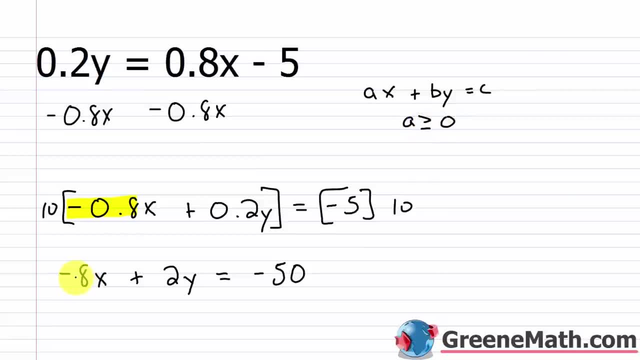 Right now I have a negative there. So how can I fix that? Well, I can multiply both sides of the equation by negative 1.. So if I multiply by negative 1, negative 1 times negative, 8x is 8x. 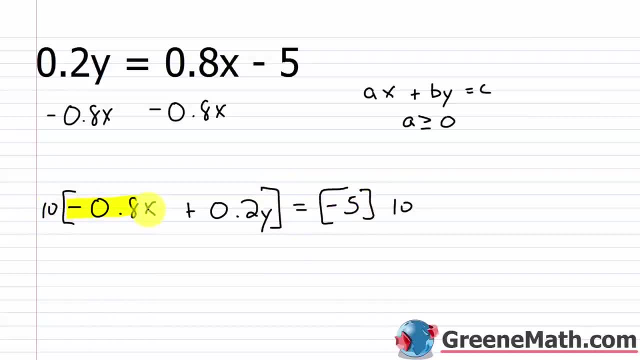 So 10 times negative 0.8x Essentially I'm just moving this one place to the right, the decimal point So this would end up being negative 8x Then plus 10 times 2y, again I'm just moving this one place to the right So this would be 2y This equals 10 times negative 5 is negative 50 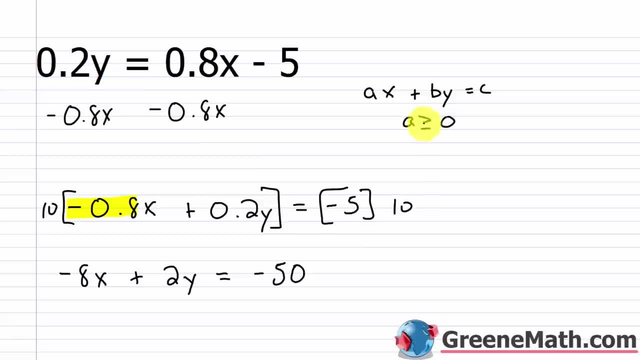 So I've solved the part where I want integers but a is not greater than or equal to 0 Right now I have a negative there So how can I fix that? Well, I can multiply both sides of the equation by negative 1 So if I multiply by negative 1 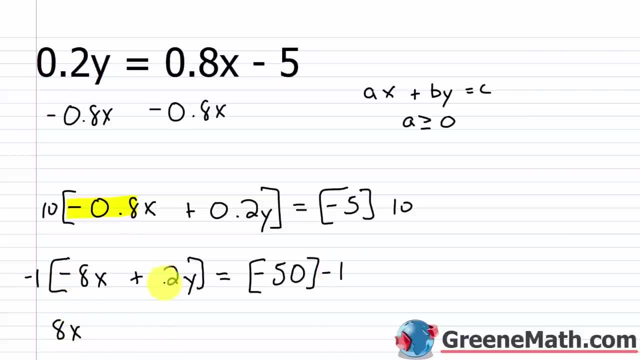 Negative 1 times negative 8x is 8x Negative 1 times 2y is minus 2y And negative 1 times negative 50 is positive 50 So now this is in standard form in the stricter form of standard form where the coefficient of x is actually positive So we have 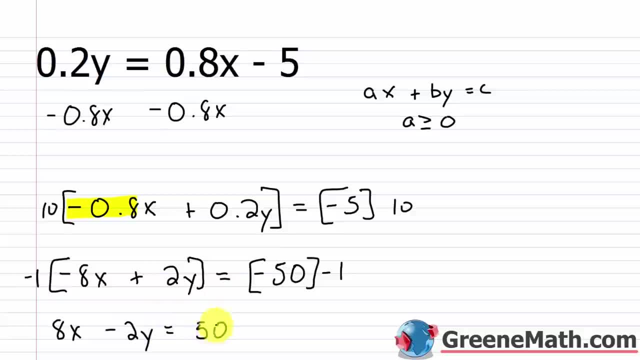 8x minus 2y equals 50 So a, b, and c are all integers 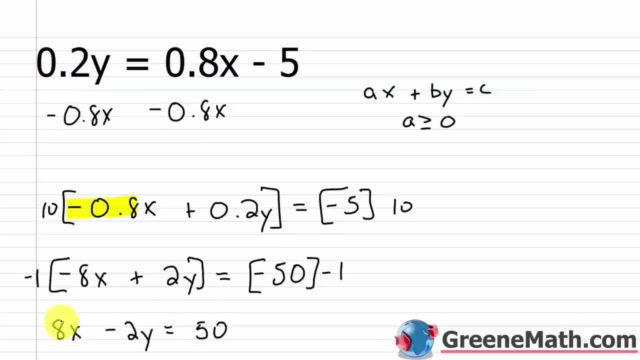 a is greater than or equal to 0 and a and b are not 0 So all of the conditions are met 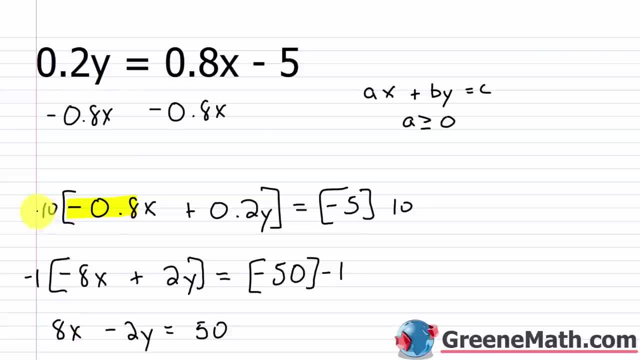 Now some of you are going to say hey you could have done that in one step I could have multiplied up here by negative 10 and I would have got this right away 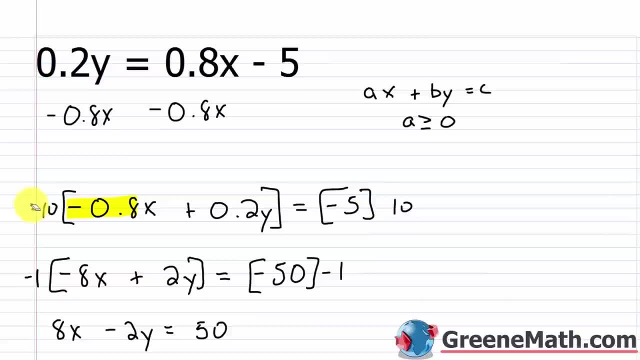 Well yes I could have done that but I wanted to make it a little easier for you to understand what we were doing so I did it in two steps 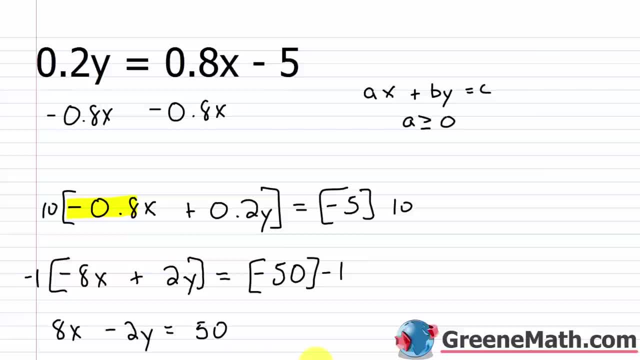 But kind of moving forward if you're looking to save time that's one of the things you might consider 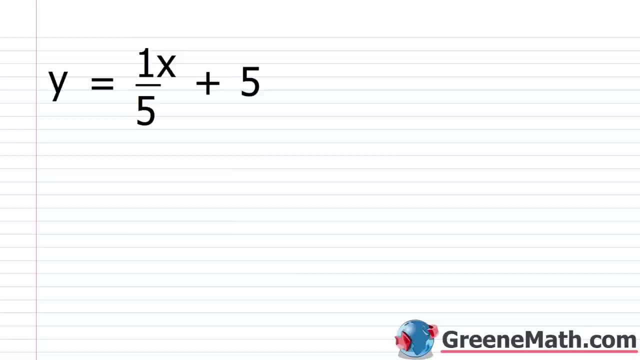 Alright, let's take a look at another one So we have y equals 1 fifth x plus 5 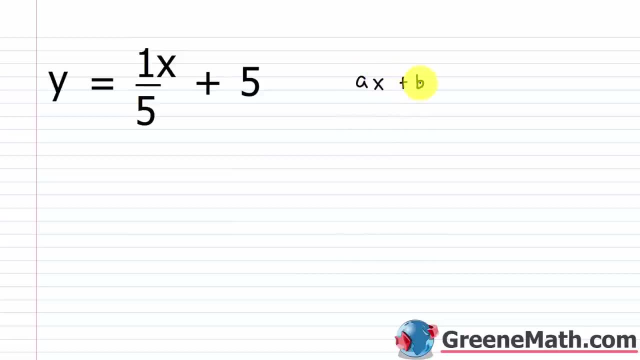 So again I'm looking for ax plus by equals c and again I want a to be greater than or equal to 0 and b to be greater than or equal to 0 I want a, b, and c to be integers and I want a and b to not both be 0 I'm going to start out by subtracting 1 fifth x away from both sides of the equation So I'd have y minus 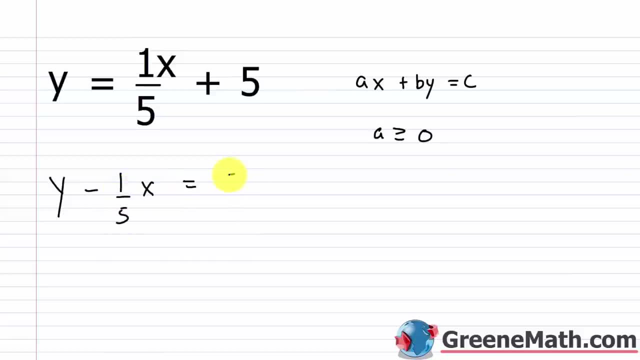 1 fifth x is equal to 5 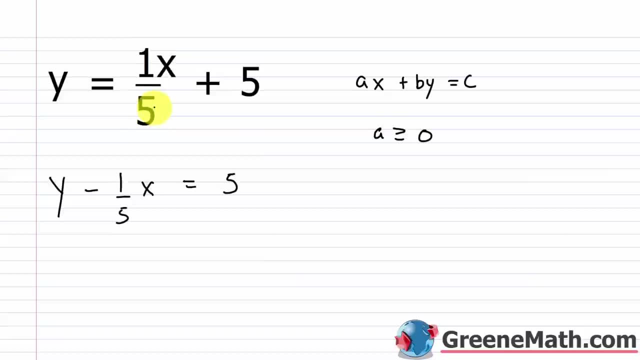 I just subtracted 1 fifth x away from here, that would make it cancel 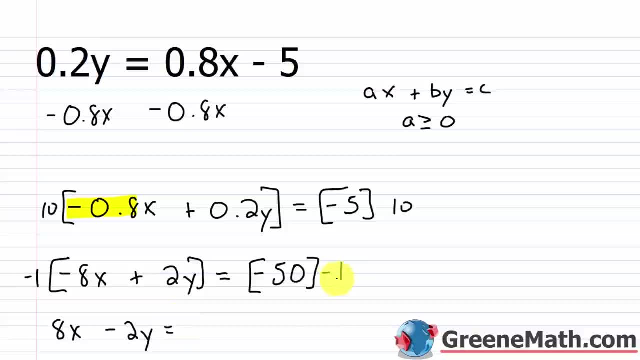 Negative 1 times 2y is minus 2y, And negative 1 times negative 50 is positive 50. So now this is in standard form, in the stricter form of standard form, where the coefficient of x is actually positive. 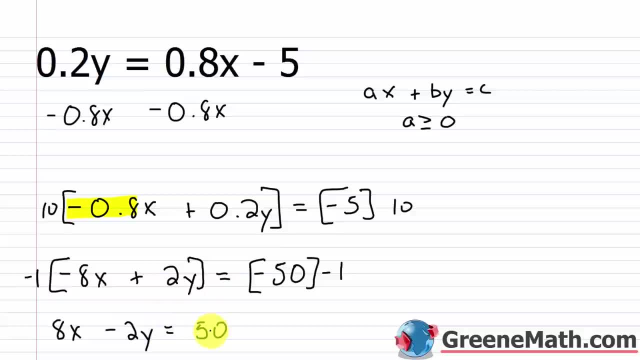 So we have 8x minus 2y equals 50. So a, b and c are all integers. a is greater than or equal to 0. And a and b are not 0. So all of the conditions are met. 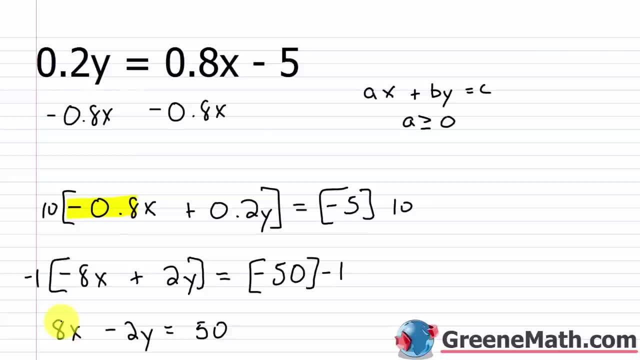 Now some of you are going to say, hey, you could have done that in one step. I could have multiplied up here by negative 10. And I would have got this. I could have done that right away. Well, yes, I could have done that. 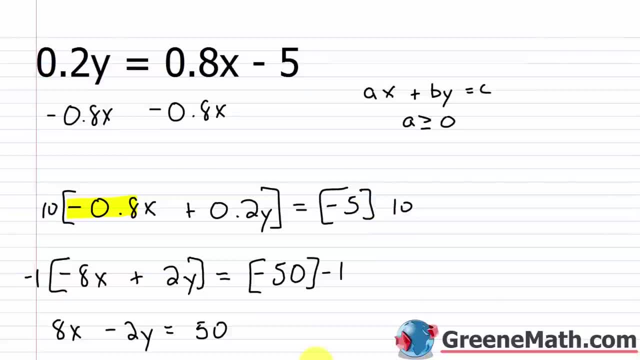 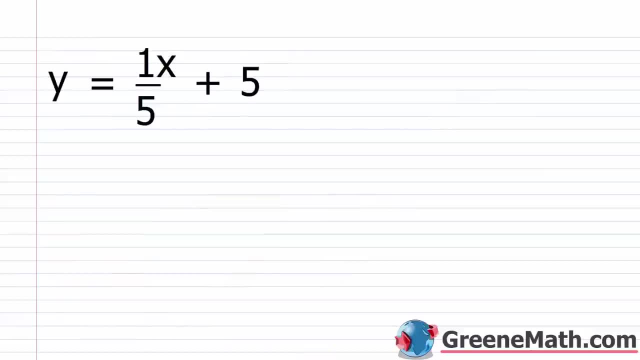 But I wanted to make it a little easier for you to understand what we were doing, So I did it in two steps, But kind of moving forward. if you're looking to save time, that's one of the things you might consider. All right, let's take a look at another one. 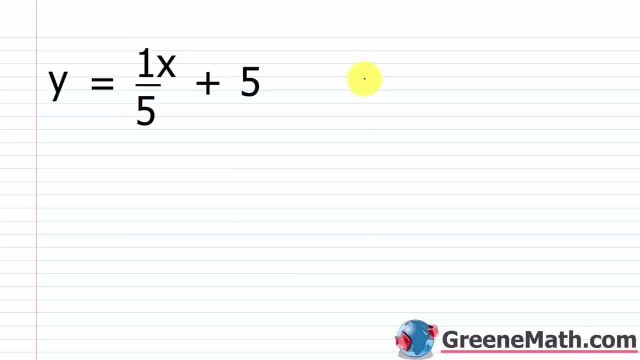 So we have y equals 1, fifth x plus 5.. So again I'm looking for ax plus by equals c, And again I want a to be greater than or equal to 0.. I want a, b and c to be integers. 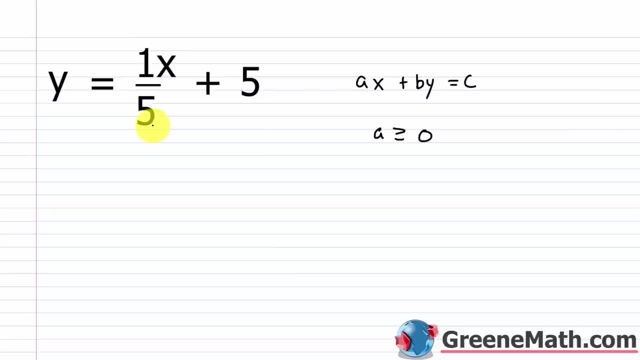 And I want a, b and c to not both be 0.. I'm going to start out by subtracting 1 fifth x away from both sides of the equation, So I'd have y minus 1 fifth x is equal to 5.. 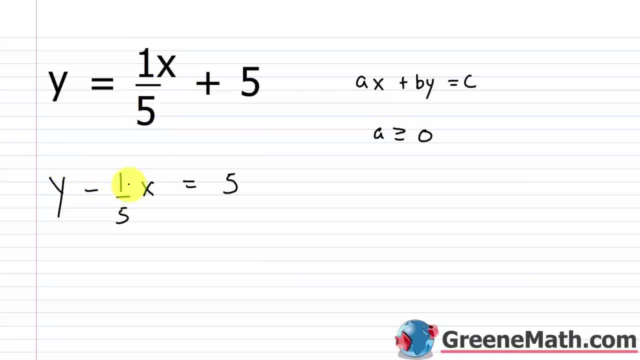 And I just subtracted 1 fifth x away from here. That would make it cancel. I subtract away from here, I have it over here In this particular case, let's think about this. Let's think about doing it in one step. 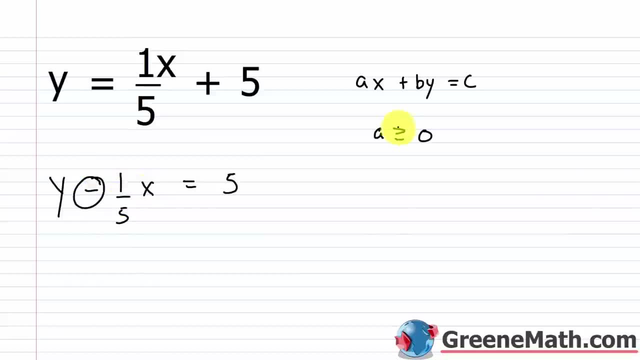 I have the fact that this is negative. I have a negative coefficient for x. It's going to specifically be greater than or equal to 0. And I have a fraction. So I don't want that either. I want an integer. So what can I multiply 1 fifth by to make it a whole number? 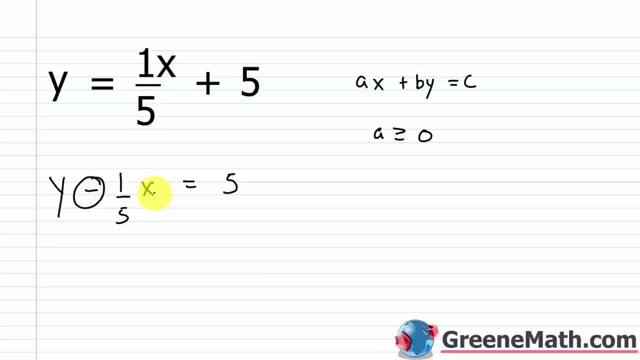 I can multiply by 5.. If I multiply 5 by 1 fifth, I get 1.. Multiply a number by its reciprocal, you get 1.. Additionally, if I threw in the fact that I multiplied by negative 5, I would change the sign here. 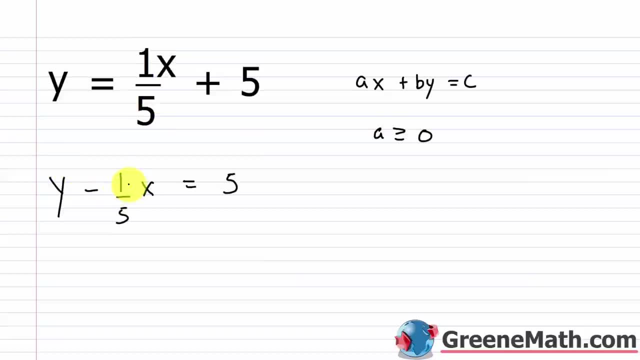 I subtract away from here, I have it over here In this particular case 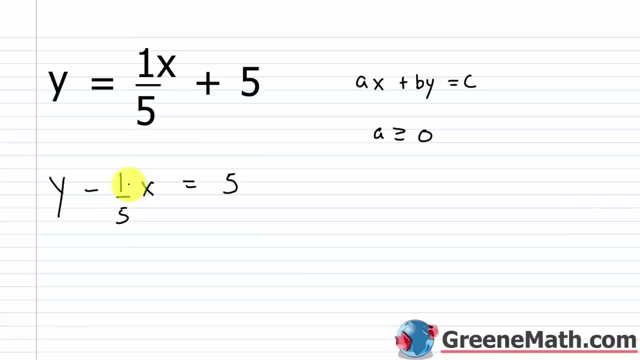 let's think about this, let's think about doing it in one step I have the fact that this is negative I have a negative coefficient for x I don't want that, a has to specifically be 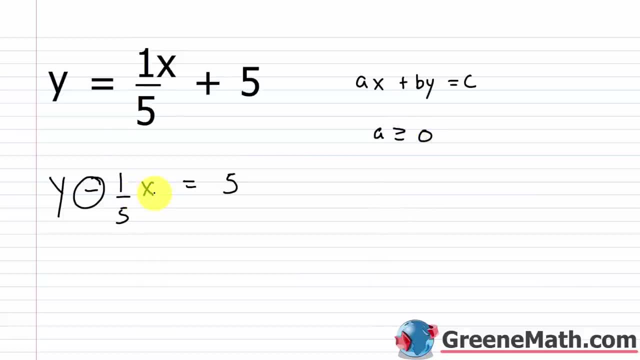 greater than or equal to 0 and I have a fraction, so I don't want that either I want an integer So what can I multiply 1 fifth by 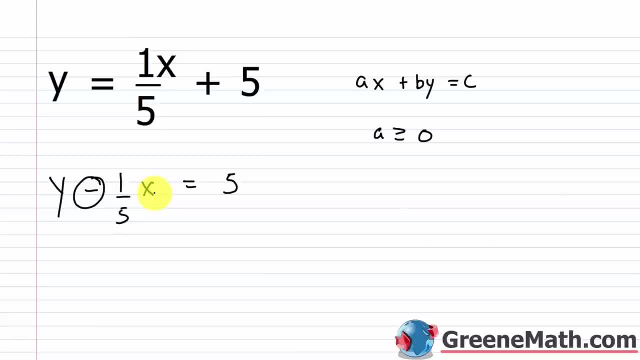 to make it a whole number I can multiply it by 5 If I multiply 5 by 1 fifth I get 1, multiply a number by its reciprocal you get 1 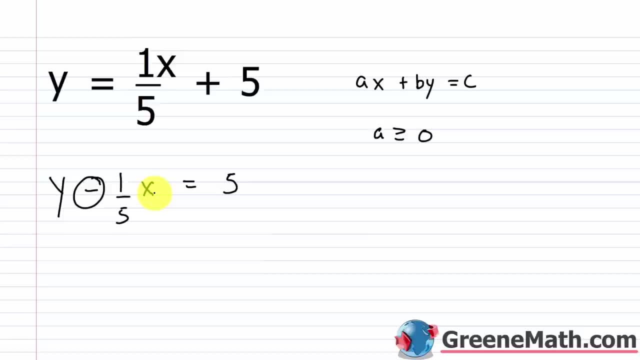 Additionally, if I threw in the fact that I multiplied by negative 5 I would change the sign here because right now we have a negative 1 fifth So if I multiply negative 1 fifth 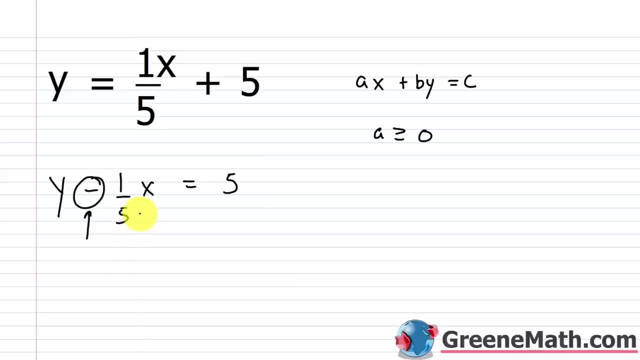 by negative 5 I solve both my problems there Again, to make that legal though I've got to do it by both sides of the equation 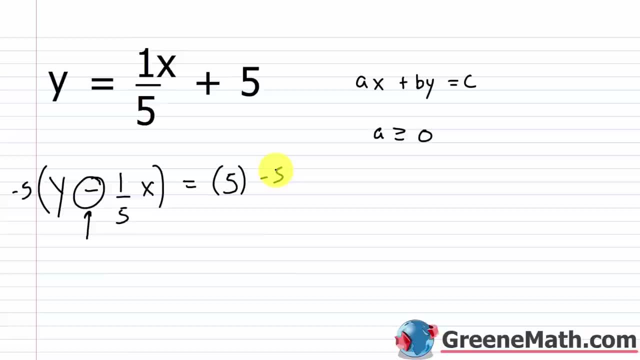 So multiply over here by negative 5 and also over here by negative 5 negative 5 times y is negative 5y negative 5 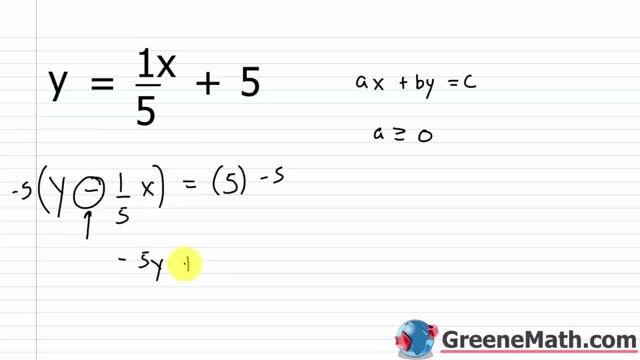 times negative 1 fifth x is going to be plus 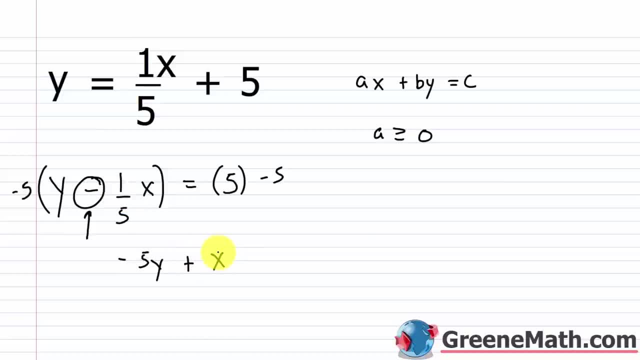 x, you can put plus 1 x if you want, it doesn't really matter 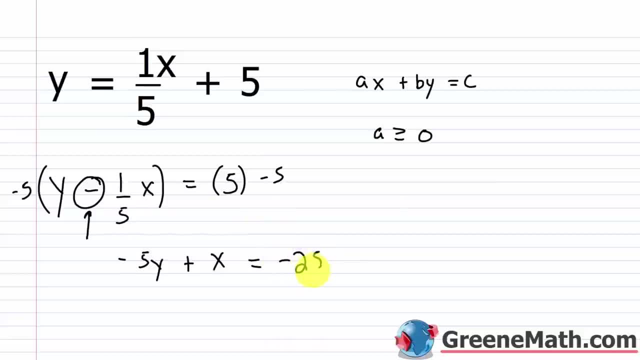 This is going to equal 5 times negative 5 which is negative 25 Now you might say, well this doesn't look like that 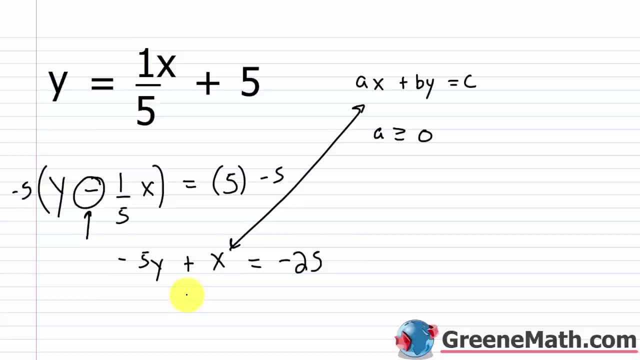 All you have to do is switch the order here Remember addition is commutative So I could rewrite this as x minus 5y 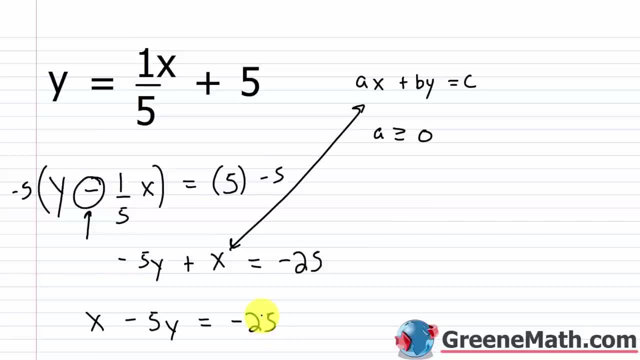 is equal to negative 25 and I've written this in standard form using the stricter definition My a term here is 1 so it's greater than or equal to 0 My b term is negative 5 My c term is negative 25 So a, b, and c are integers a is greater than or equal to 0 and neither of them are 0 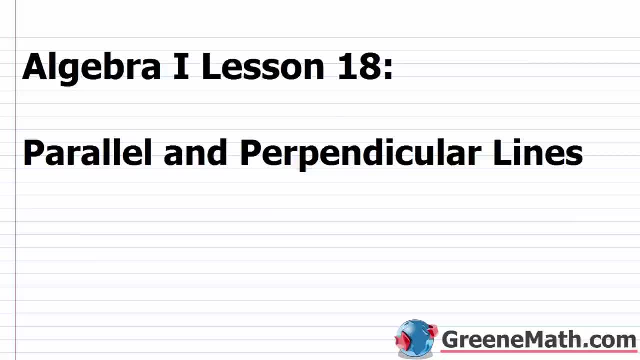 Hello and welcome to Algebra 1 Lesson 18 In this video we're going to learn about parallel and perpendicular lines So parallel lines are any two lines on a plane 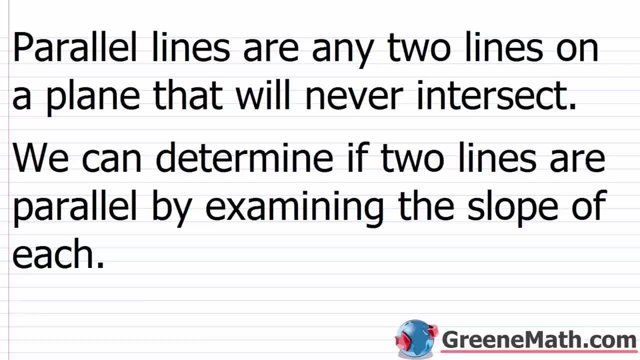 that will never intersect We can determine if two lines 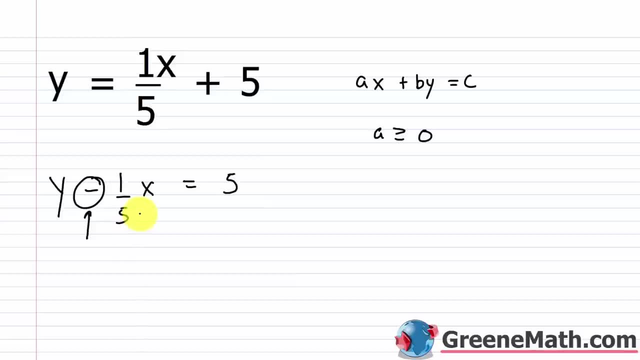 Because right now we have a negative 1 fifth. So if I multiply Negative 1 fifth by negative 5, I solve both my problems there. Again, to make that legal, though, I've got to do it by both sides of the equation. 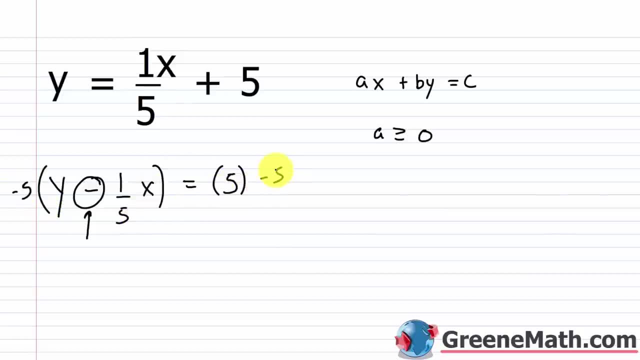 So multiply over here by negative 5 and also over here by negative 5.. Negative 5 times y is negative 5y. Negative 5 times negative: 1. fifth, x is going to be plus x. You can put plus 1 x if you want. 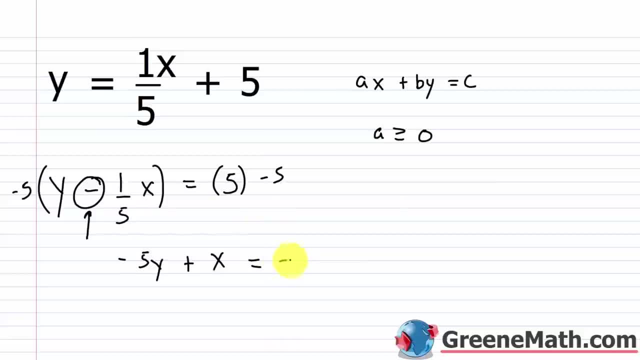 It doesn't really matter. And this is going to equal 5 times negative 5, which is negative 25.. Now you might say: Well, This doesn't look like that. All you have to do is switch the order here. 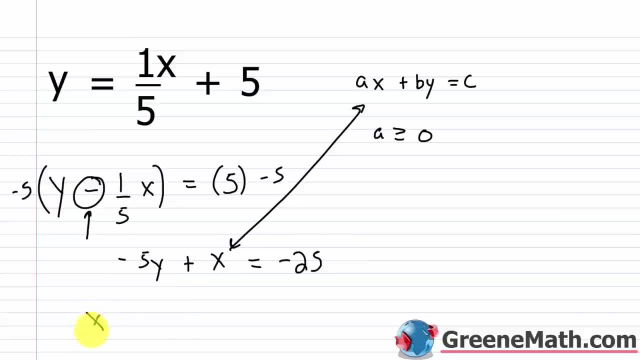 Remember, addition is commutative, So I could rewrite this as: x minus 5y is equal to negative 25.. And I've written this in standard form using the stricter definition right. My a term here is 1.. So it's greater than or equal to 0.. 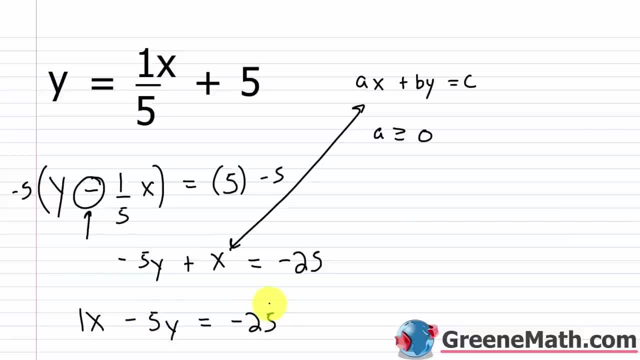 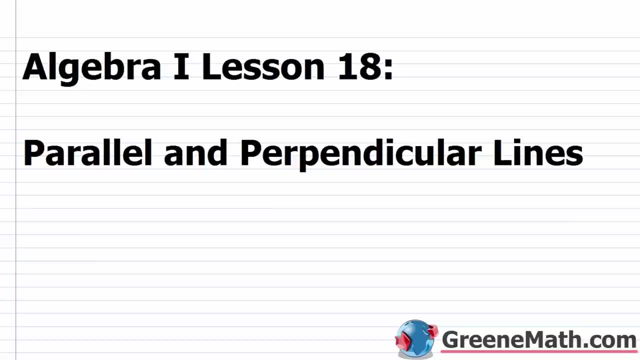 My b term is negative 5.. My c term is negative 25.. So a, b and c are integers. a is greater than or equal to 0. And a and b are not both 0. Right, So I'm going to write this down. 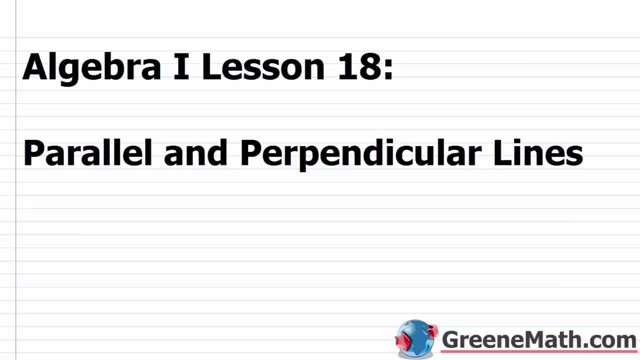 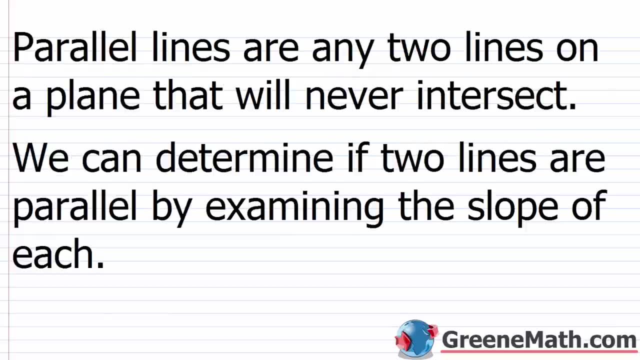 Hello and welcome to Algebra 1, Lesson 18.. In this video we're going to learn about parallel and perpendicular lines. So parallel lines are any two lines on a plane that will never intersect. We can determine if two lines are parallel by examining the slope of each. 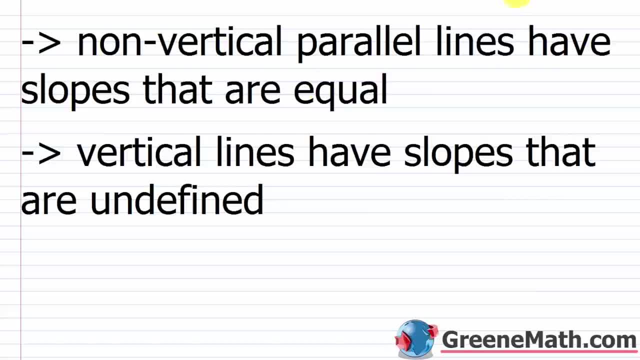 So non-vertical parallel lines have slopes that are equal. Let me highlight that Non-vertical parallel lines have slopes that are equal. Okay, Very important that you write that down Now. vertical lines, remember, they have slopes that are undefined. So that's why we specify and say that non-vertical parallel lines have slopes that are equal. 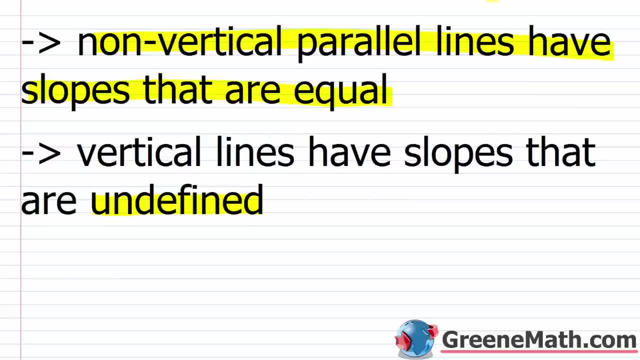 But vertical lines have slopes that are undefined. Now, when you first start looking at parallel lines, what you're going to notice is that there are lines that kind of look the same. So parallel lines look like this. Let's say, I had a line that goes this way and another line that looked like that. 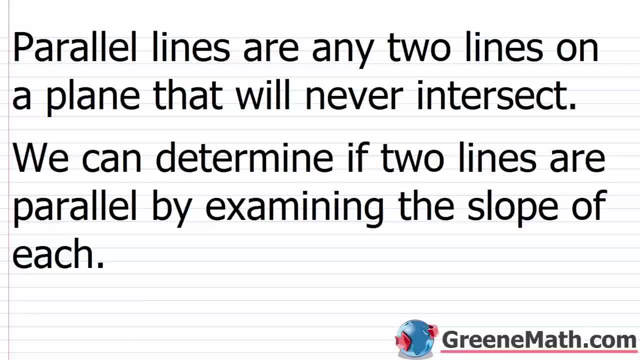 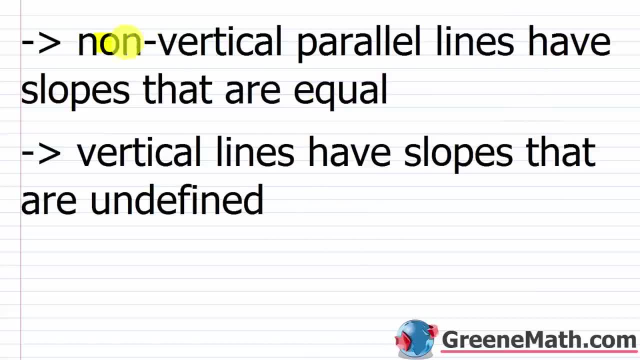 are parallel by examining the slope of each So non-vertical parallel lines have slopes that are equal Let me highlight that Non-vertical parallel lines have slopes that are equal 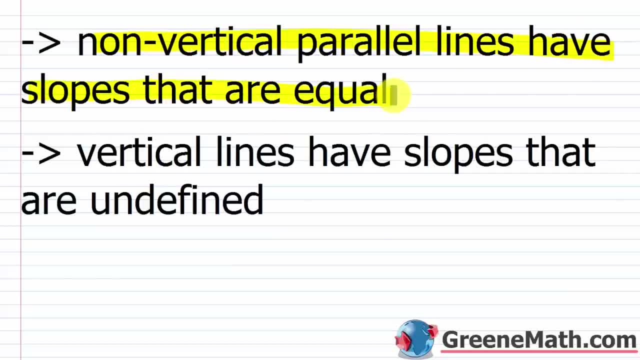 Very important that you write that down Now vertical lines remember they have slopes that are undefined So that's why we specify and say that non-vertical parallel lines 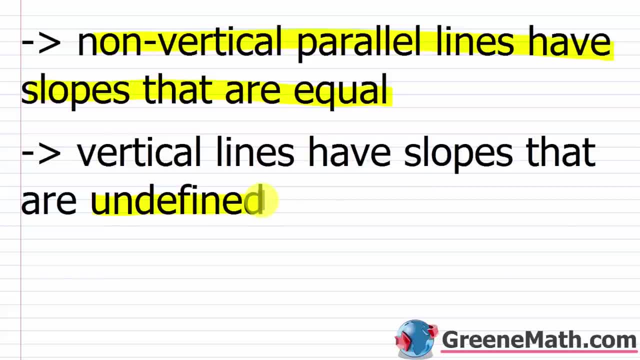 have slopes that are equal but vertical lines have slopes that are undefined 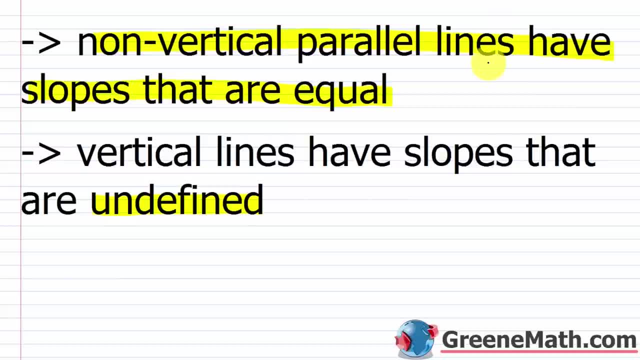 Now when you first start looking at parallel lines what you're going to notice is that there are lines that kind of look the same So parallel lines look like this Let's say I had a line that goes this way like that So I know these aren't perfect but you can see by looking at these lines that they're never going to intersect 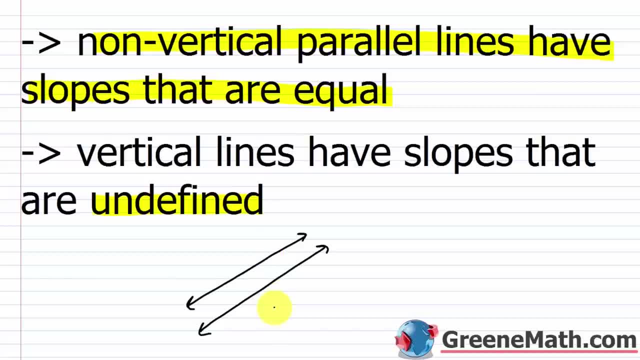 And if we're on a coordinate plane you'd also see that they have different y-intercepts 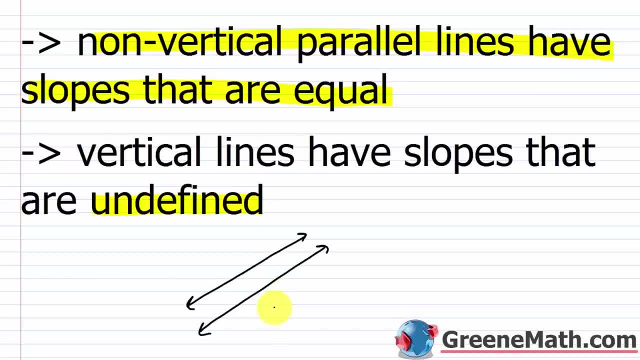 So essentially you're looking for same slope, different y-intercepts those are going to be parallel lines 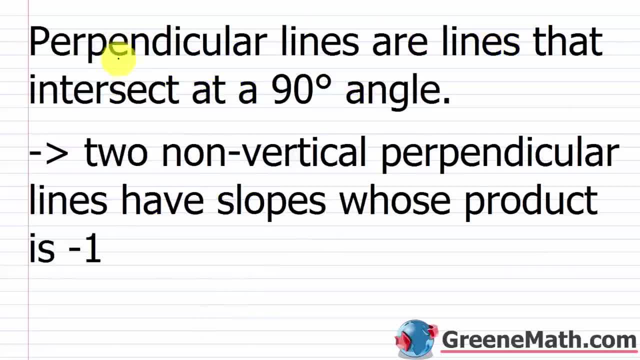 So then the other thing we want to talk about 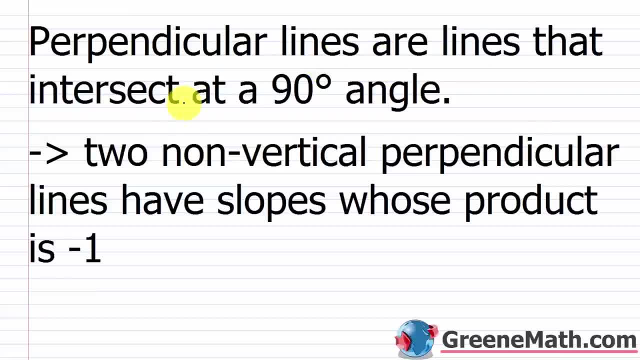 are perpendicular lines And perpendicular lines are lines that intersect at a 90 degree angle 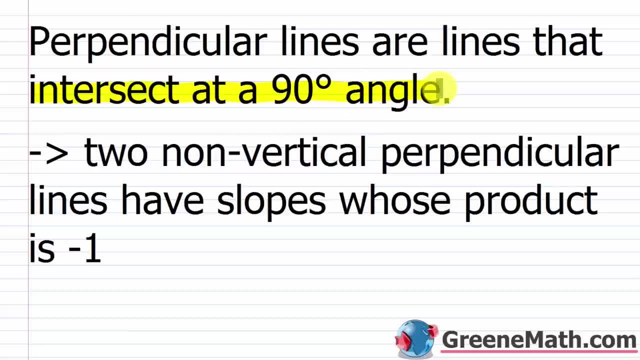 They intersect at a 90 degree angle 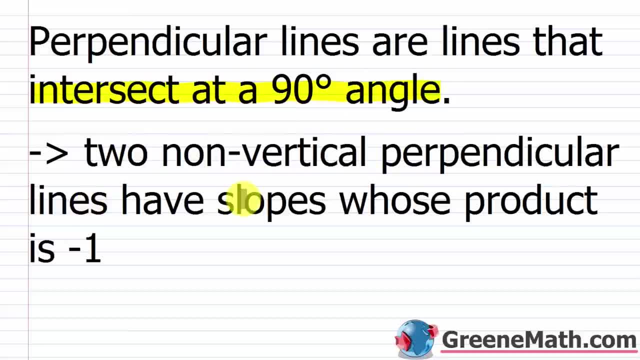 So two non-vertical perpendicular lines have slopes whose product whose product is negative one 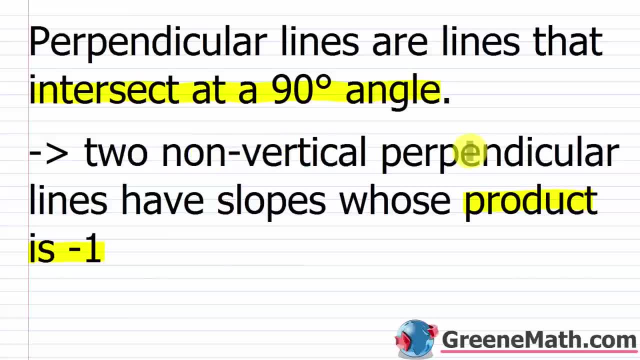 So specifically if I take two non-vertical perpendicular lines and I grab their slopes I multiply them together the result is always going to be negative one 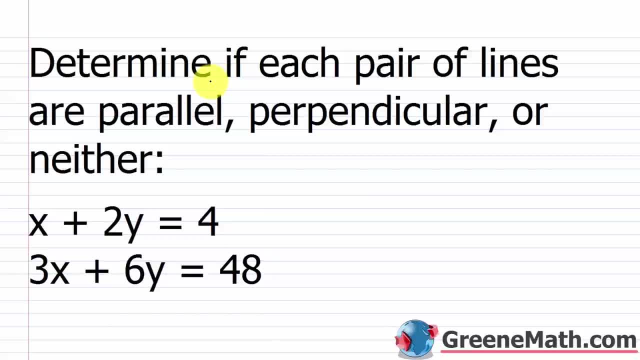 So we're going to look at a few examples here Not really a difficult concept whatsoever So we want to determine 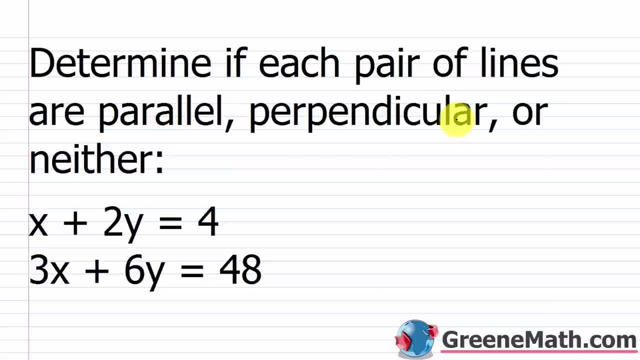 if each pair of lines is parallel, perpendicular or neither 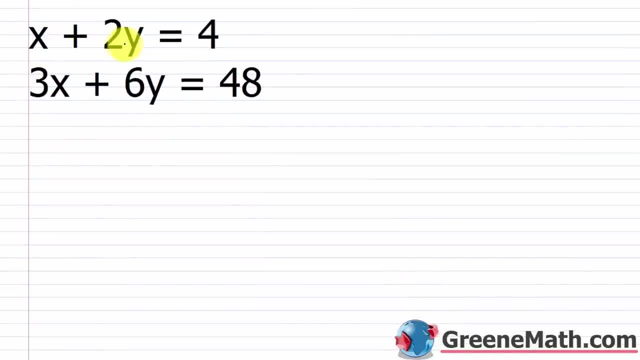 So let's start out with x plus 2y equals 4 and then 3x plus 6y equals 48 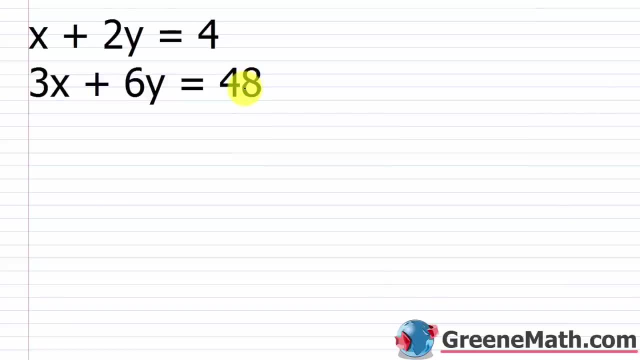 So when you get problems like this for your homework or for a test the first thing you want to do is find the slope of each line Now, we found out in the last lesson that an easy way to do that was to put your line in what's called 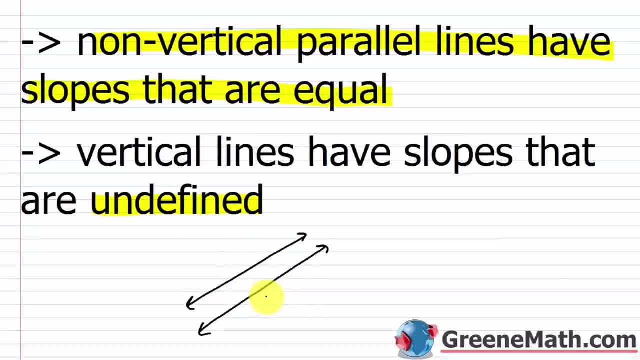 So I know these aren't perfect, but you can see by looking at these lines that they're never going to intersect, And if we're on a coordinate plane, you'd also see that they have different y-intercepts. So essentially you're looking for same slope, different y-intercepts. 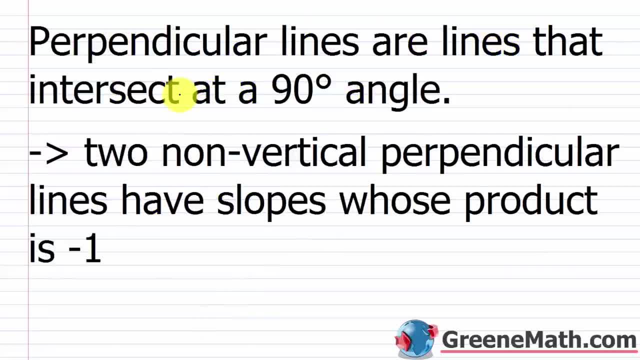 Those are going to be parallel lines. So then, the other thing we want to talk about are perpendicular lines, And perpendicular lines are lines that intersect at a 90 degree angle. Okay, They intersect at a 90 degree angle. So two non-vertical perpendicular lines have slopes. whose product? okay, whose product? 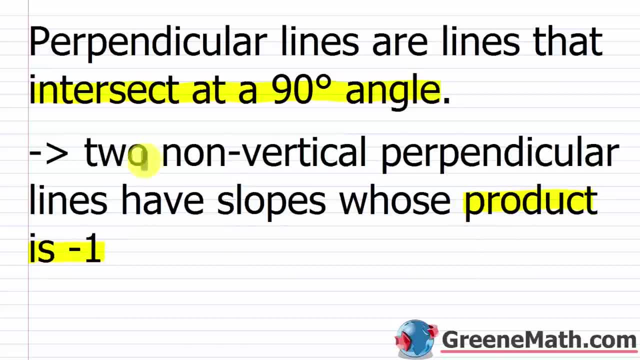 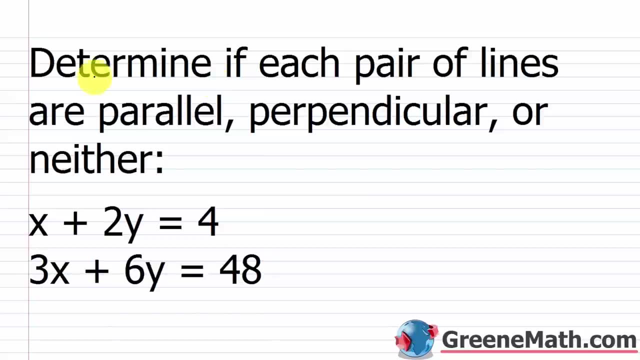 is negative 1.. So, specifically, if I take two non-vertical perpendicular lines and I grab their slopes, I multiply them together, the result is always going to be negative 1.. So we're going to look at a few examples here. Not really a difficult concept whatsoever. 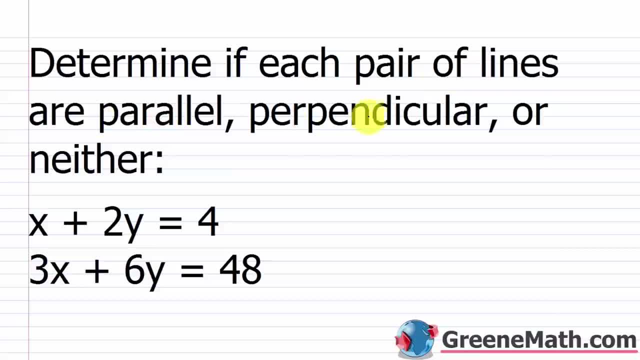 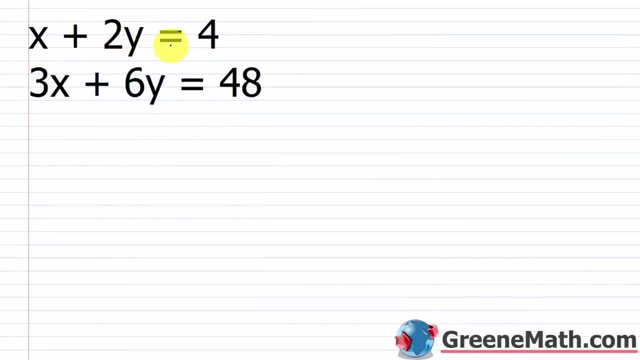 So we want to determine if each pair of lines are parallel, Perpendicular or neither. Okay, So let's start out with: x plus 2y equals 4.. And then 3x plus 6y equals 48. So when you get problems like this for your homework or for a test, the first thing you 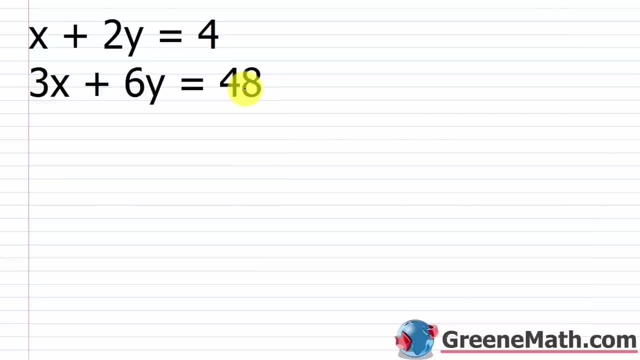 want to do is find the slope of each line. Now we found out in the last lesson that an easy way to do that was to put your line in what's called slope-intercept-intercept, And basically that means you're going to put your line in the format of y is equal. 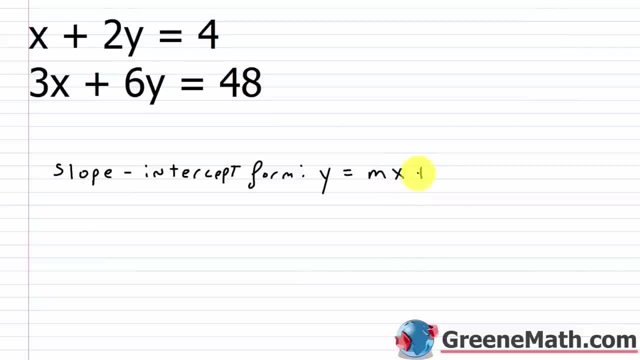 to m the slope times, x plus b the y-intercept. This is the slope and this is the y-intercept. That's why it's called slope-intercept-form. So, essentially, what you have to do is just take each equation and solve it for y. 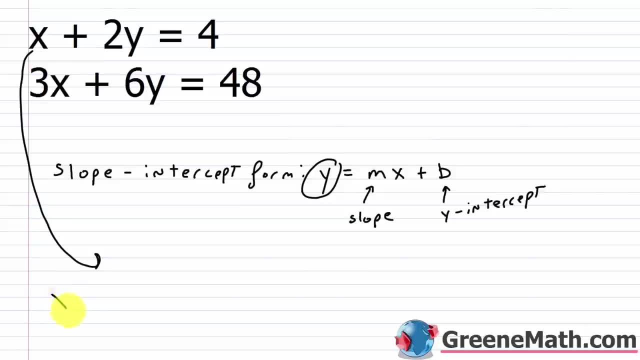 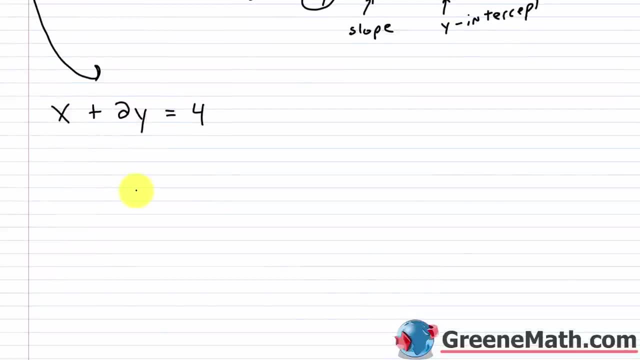 That's all you need to do, So I'll start out with this. x plus 2y is equal to 4. And I'm going to solve this for y. So in order to do that, I'm going to subtract x away from each side of the equation. 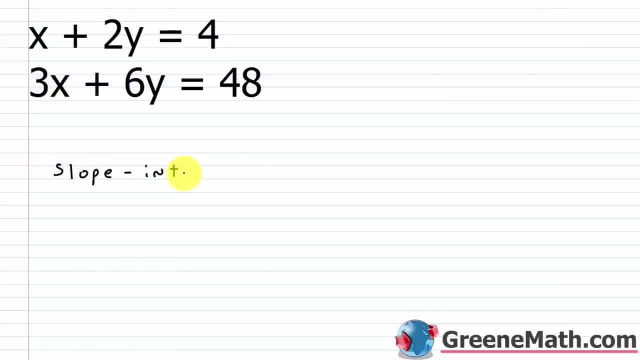 slope intercept form And basically that means you're going to put your line in the format of y is equal to m the slope times x 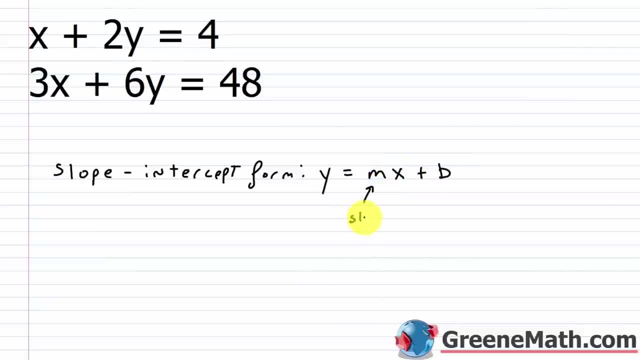 plus b the y intercept This is the slope and this is the y intercept 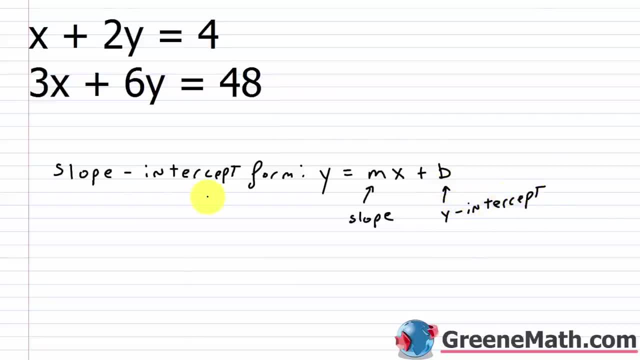 That's why it's called slope intercept form 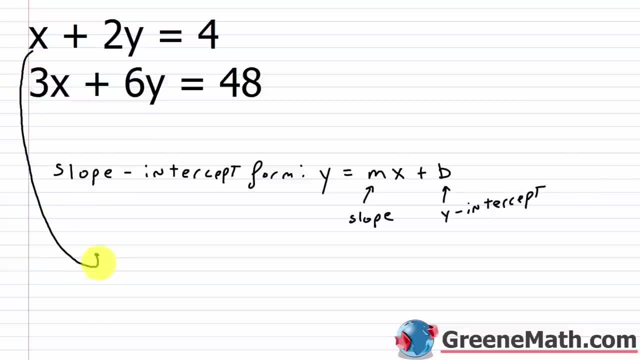 So essentially what you have to do is just take each equation and solve it for y and that's what you need to do 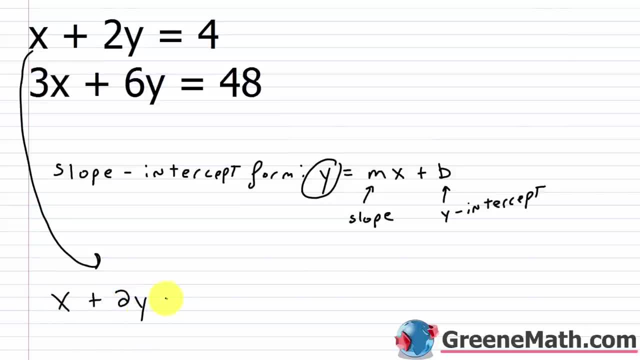 So I'll start out with this x plus 2y is equal to 4 and I'm going to solve this for y So in order to do that I'm going to subtract 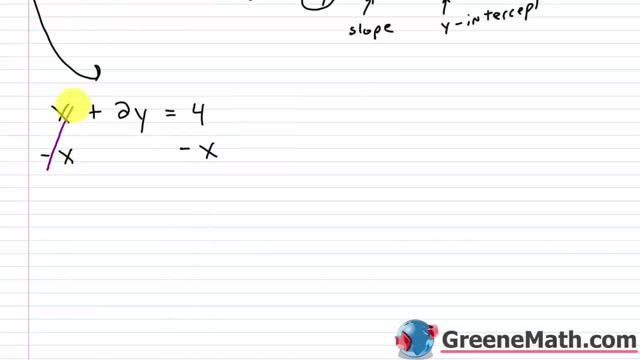 x away from each side of the equation So that's going to go away from over here and then on the left I'm just left with 2y and this is equal to I now have negative x on the right and then plus 4 I want y by itself and what's stopping me is I have this 2 So I need to divide by 2 on this side of the equation and to make it legal I need to do it to this side of the equation as well But remember we're allowed to break this up and divide 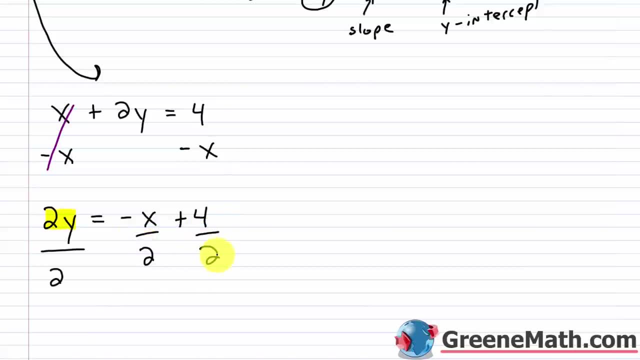 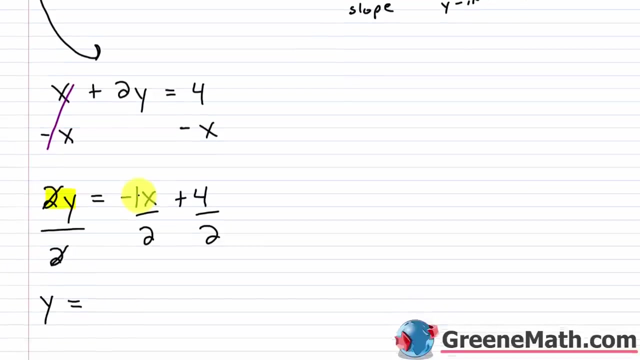 each by 2 Alright So then this would cancel with this leaving me with just y over here Over here I have negative x over 2. Remember I can always put a 1 here and say that's negative 1 times x It's kind of an invisible co-efficient if you just have a negative out in front or nothing out in front you could say hey if this is a negative out in front it's really negative 1 if there's nothing out in front it's just a 1 Alright so I can think of this as negative 1 half 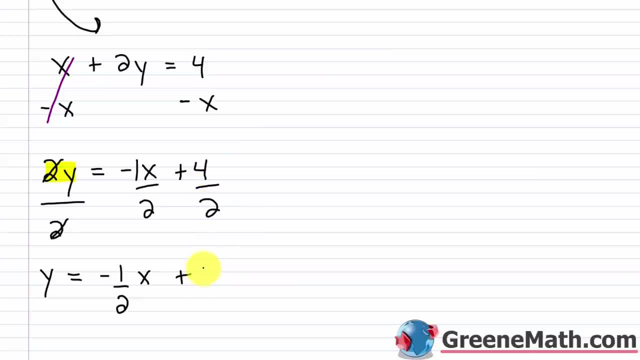 times x plus 4 over 2 is just 2 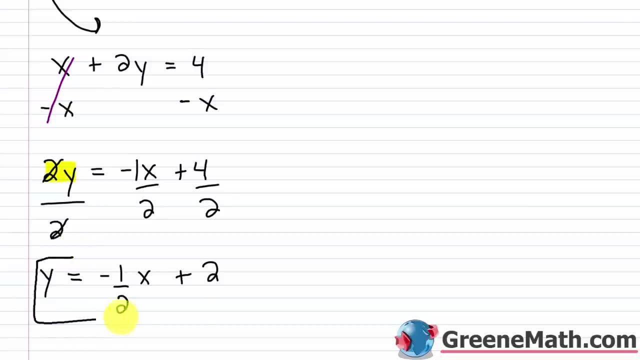 So there is my first equation in slope intercept form 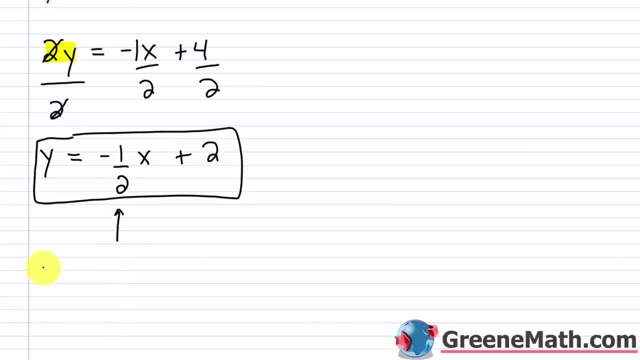 So what we can tell is that our slope which we denote as m is going to be negative 1 half and our y intercept 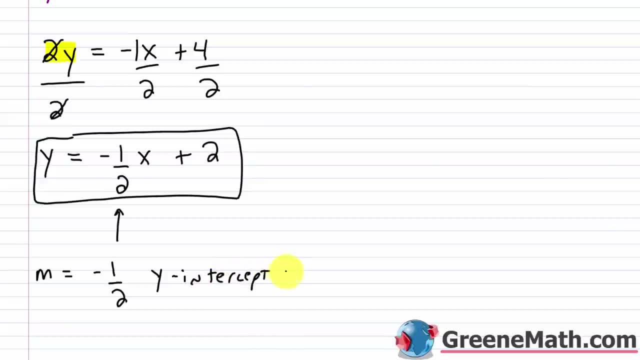 our y intercept occurs at the point 0 comma 2 Ok 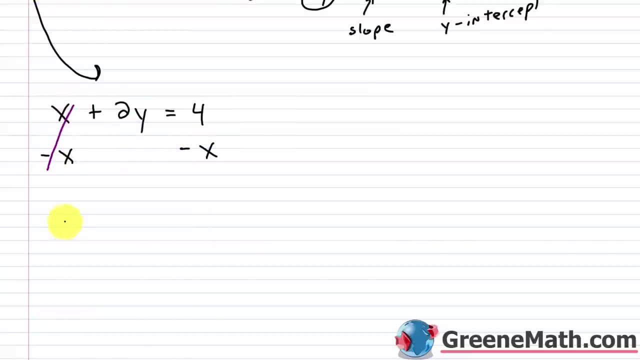 So that's going to go away from over here. And then on the left, I'm just left with 2y And this is equal to. I now have negative x on the right And then plus 4.. I want y by itself. 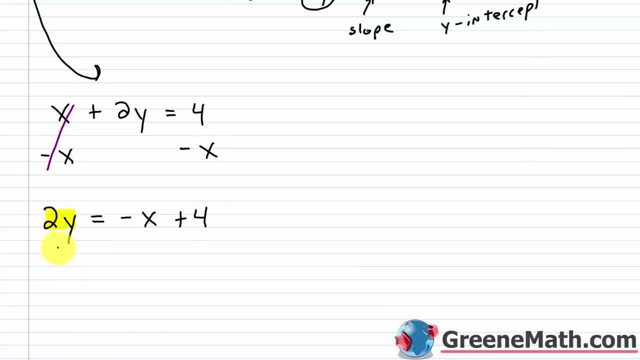 And what's stopping me is I have this: 2 that's multiplying y, So I need to divide by 2 on this side of the equation And to make it legal, I need to do it to this side of the equation as well. 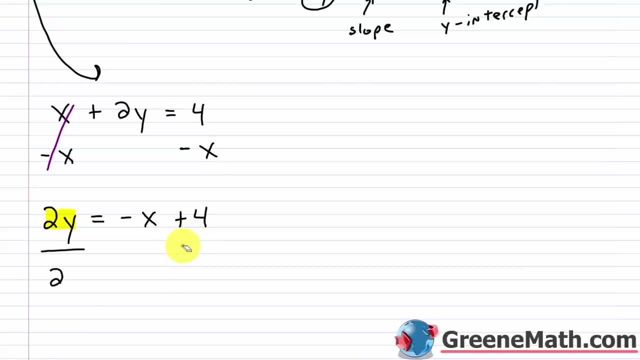 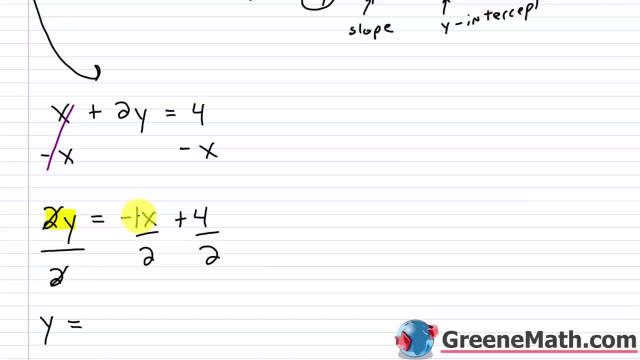 Right, Right, Right. This is a negative out in front or nothing out in front. You could say, hey, if this is a negative out in front, it's a negative 1.. If there's nothing out in front, it's just a 1.. 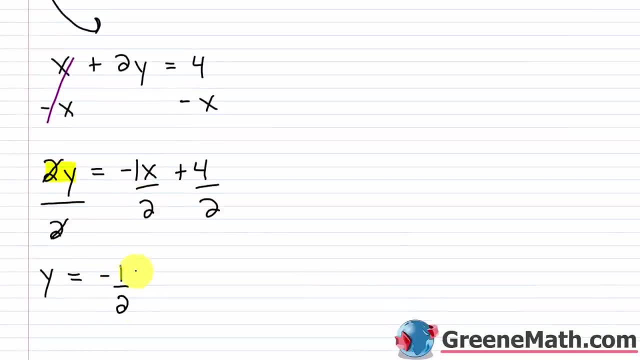 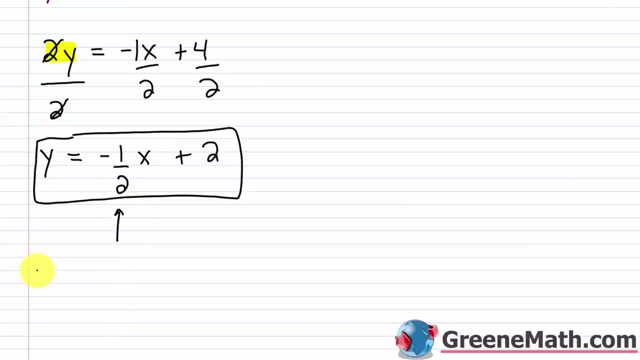 Right. So I can think of this as negative one-half times x plus 4 over 2 is just 2.. So there is my first equation in slope intercept form. So what we can tell is that our slope, which we denote as m, is gonna be negative one-half. 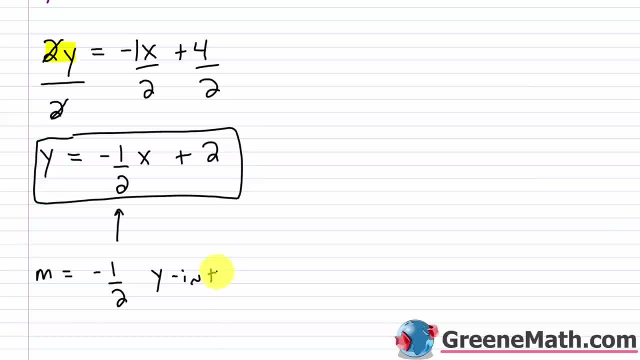 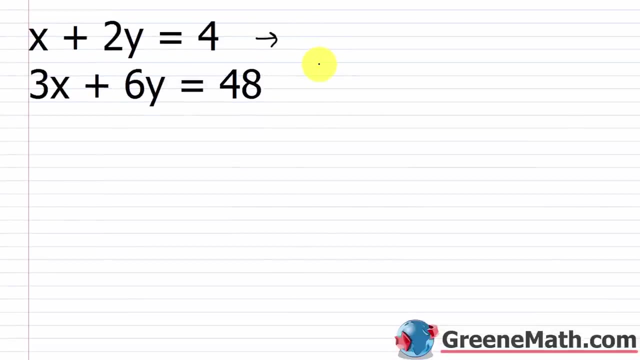 and our y intercept intercept. our y intercept occurs at the point 0, comma 2.. Okay, let's erase everything and go back up to the top. I'm just going to keep this information right here. So for this first one, again in slope intercept form, we end up with: y equals negative 1 half x plus 2.. And again we 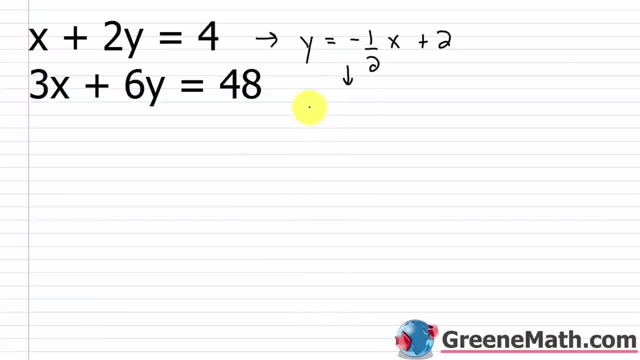 said that this corresponds to a slope which is m equal to negative 1 half and a y intercept, a y intercept that occurs at the point 0, comma 2.. All right, let's take a look at this equation now and again. all we're going to do is solve it for y. So we have 3x plus 6y equals 48.. Okay, so if I Let's erase everything and go back up to the top 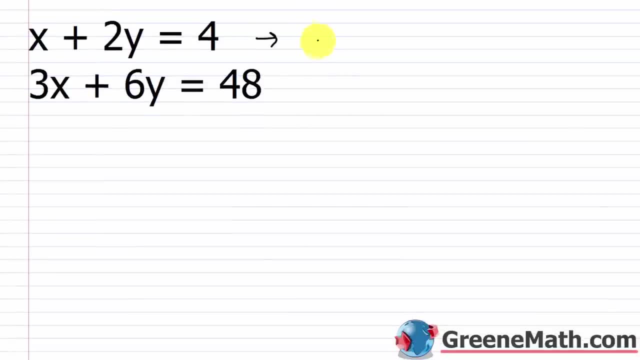 I'm just going to keep this information right here So for this first one again in slope intercept form we end up with y equals negative 1 half x plus 2 and again we said that this corresponds to a slope which is m equal to negative 1 half and a y intercept a y intercept that occurs at the point 0 comma 2 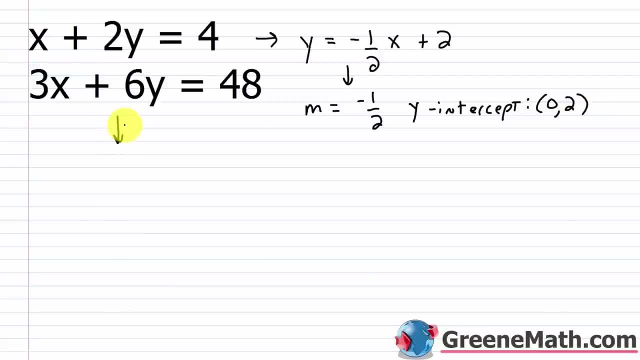 Alright let's take a look at this equation now and again all we're going to do is solve it for y So we have 3x plus 6y equals 48 Ok so if I want y by itself I've got to first isolate the term 6y So I would subtract 3x away from both sides of the equation and this is going to cancel On the left now I just have 6y and this is equal to negative 3x plus 48 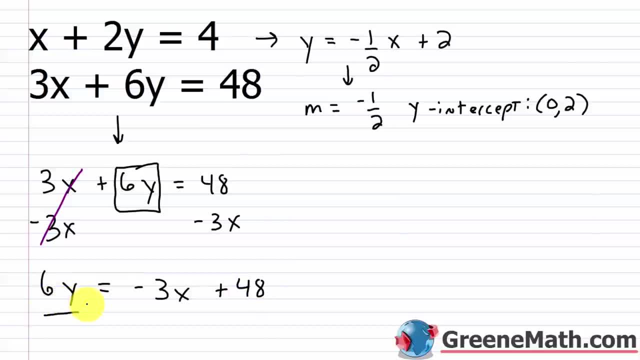 In order to get y by itself I need to divide both sides of the equation by 6 which is the coefficient of y So I'm going to divide this by 6 and also this by 6 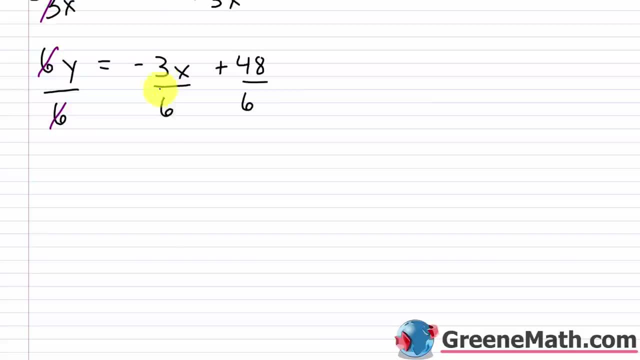 Alright so this is going to cancel with this and negative 3 over 6 is the same thing as negative 1 half I'm going to cancel this with this I'll put a 1 here and a 2 here and then 48 divided by 6 we know that's going to be 8 So I'll kind of cancel this with this and just put an 8 and a 1 So we're going to rewrite this as 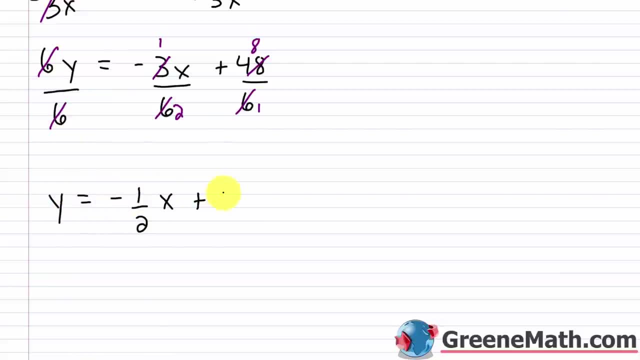 y equals negative 1 half x plus 8 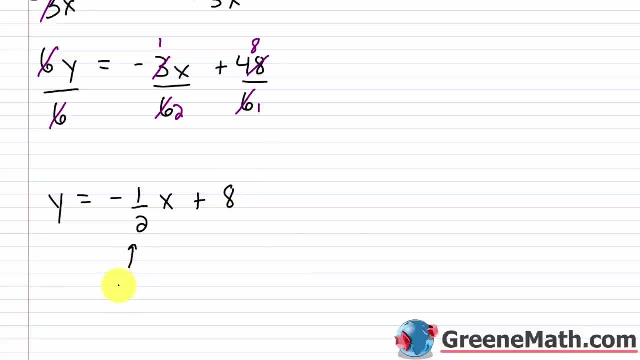 What you can immediately see is that the slope, again which is m is the same as in the other equation, it's negative 1 half The y intercept however is different, so the y intercept is going to occur at 0 comma 8 So this is your y intercept 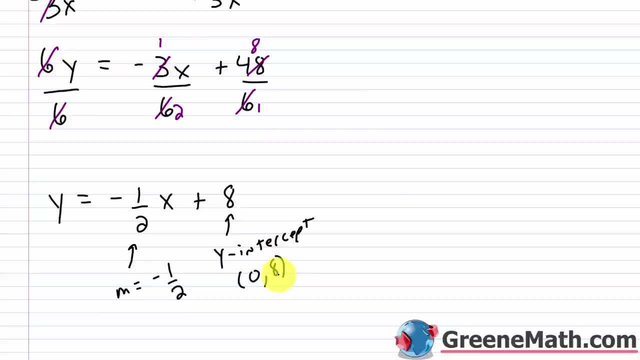 it occurs at 0 comma 8 that point on the graph So let's erase this 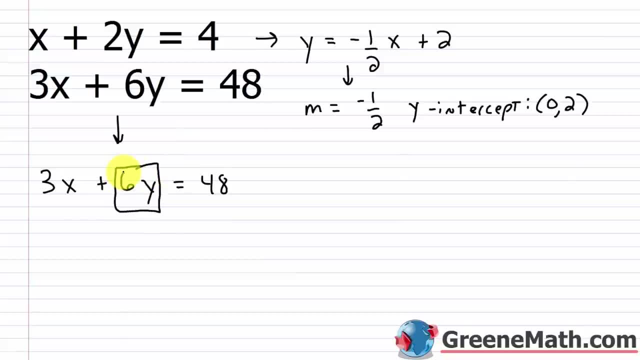 want y by itself, I've got to solve it for y. So we have: 3x plus 6y equals 48.. Okay, so if I want y by itself, I've got to first isolate the term 6y. So I would subtract 3x away from both sides of the equation and this: 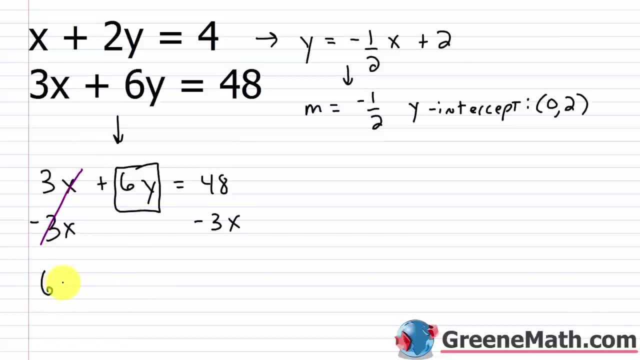 is going to cancel On the left. now I just have 6y and this is equal to negative 3x plus 48.. In order to get y by itself, I need to divide both sides of the equation by 6, which is the coefficient. 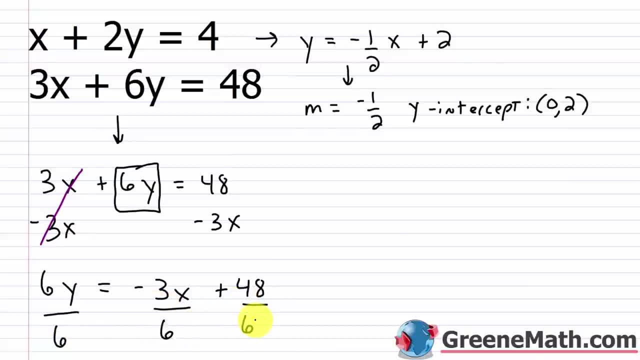 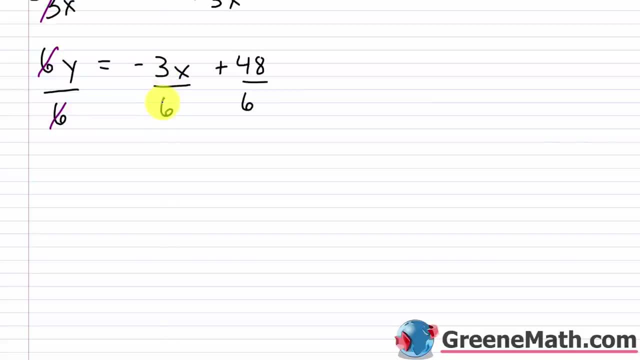 of y, So I'm going to divide this by 6 and also this by 6.. All right, so this is going to cancel with this. And negative 3 over 6 is the same thing as negative 1 half, So I'll cancel this with this. I'll put a 1 here and a 2 here. 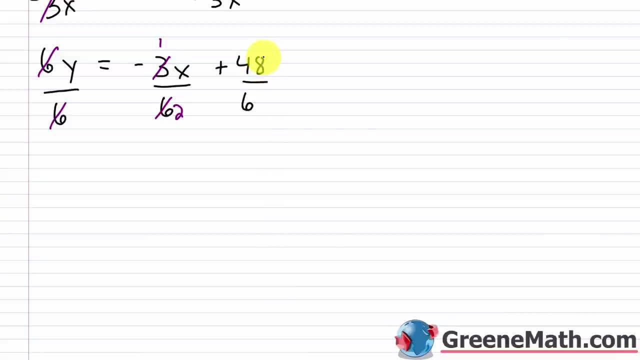 And then 48 divided by 6, we know that's going to be 8.. So I'll kind of cancel this with this and just put an 8 and a 1.. So we're going to rewrite this as y equals negative 1 half x plus 8.. What you can immediately see is that the slope 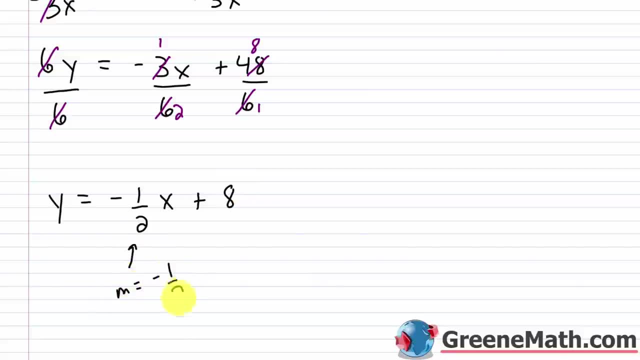 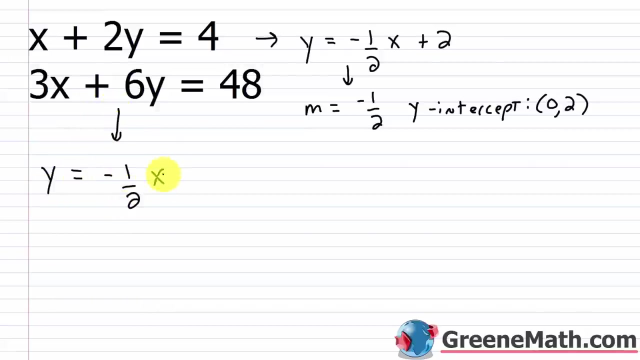 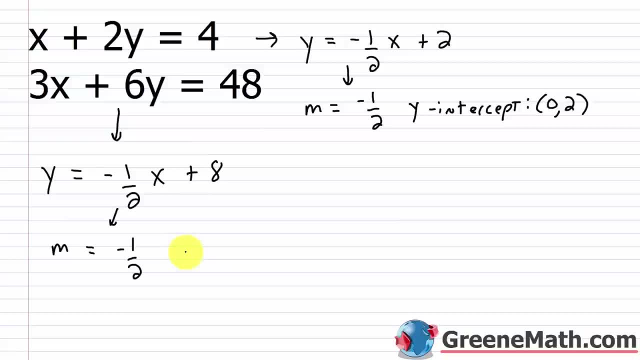 situation is also negative one half. and then the y intercept. the y intercept- let me kind of erase that real quick- is going to occur at zero comma eight. so what we can immediately tell is that we have the same slope in each case right: m equals negative one half, m equals negative one half. so 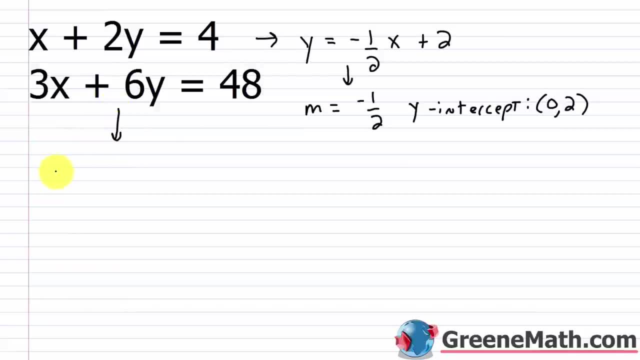 and go back up So for this line again in slope intercept form it's y equals negative 1 half x plus 8 And again m in this situation is also negative 1 half and then the y intercept the y intercept let me kind of erase that real quick 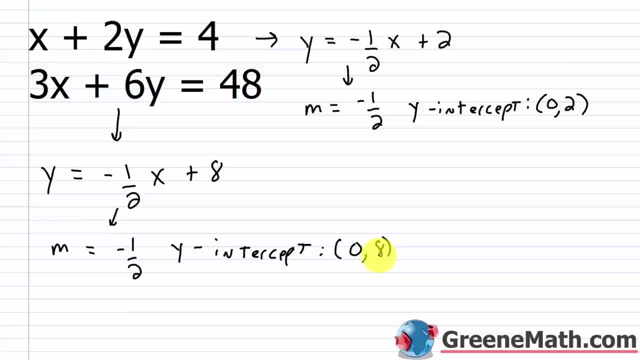 is going to occur at 0 comma 8 So what we can immediately tell is that we have the same slope 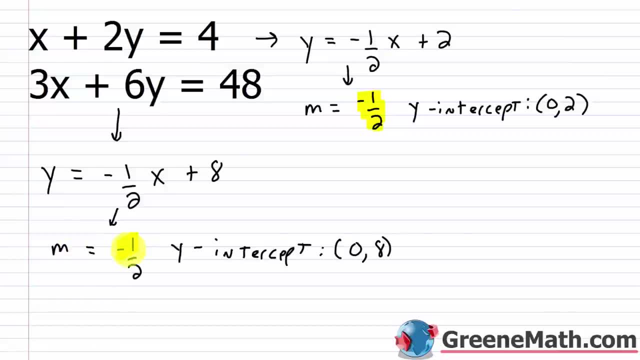 in each case, m equals negative 1 half m equals negative 1 half So same slope different y intercepts different y intercepts we know that we have parallel lines these lines are parallel 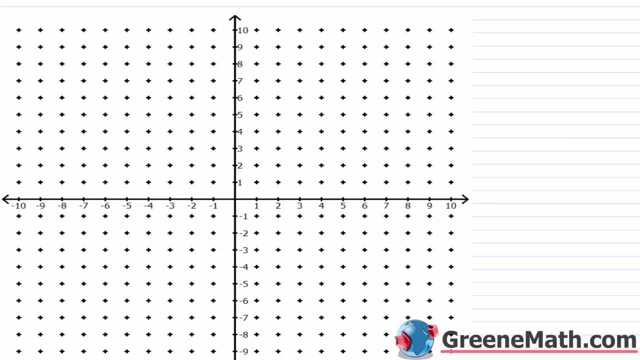 So one thing I want to show you really quickly is what this visually looks like using a coordinate point. So remember we had y equals negative 1 half x plus 2 and we had y equals 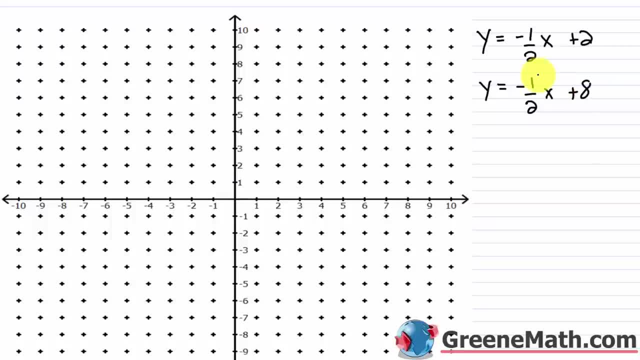 negative 1 half x plus 8 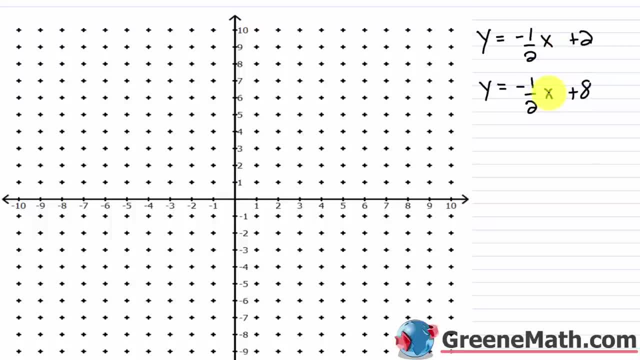 In slope intercept form we have two lines Now if we know a point on the line 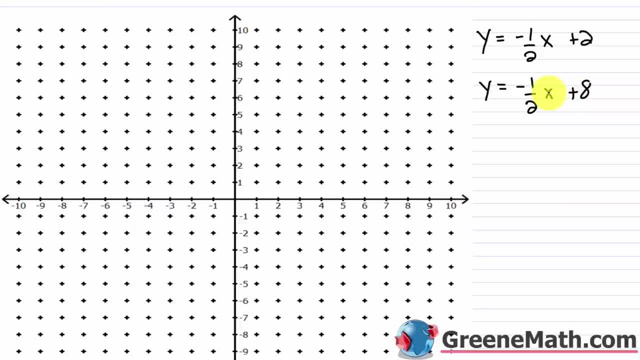 and the slope we can easily graph Remember we've kind of transcended the point where we have to go through and make ordered pairs and do all this stuff we can graph really quickly now 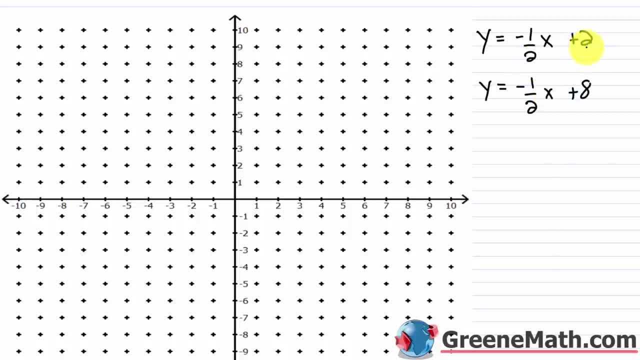 So I know for this first one the y intercept occurs at 0 comma 2 So on the coordinate plane that's going to be right here and then my slope is negative 1 half 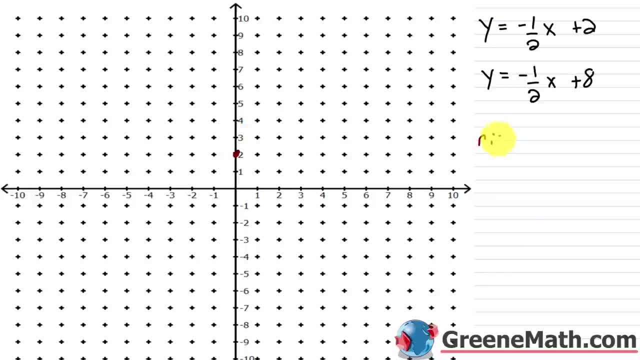 So remember it's rise over run It's rise over run 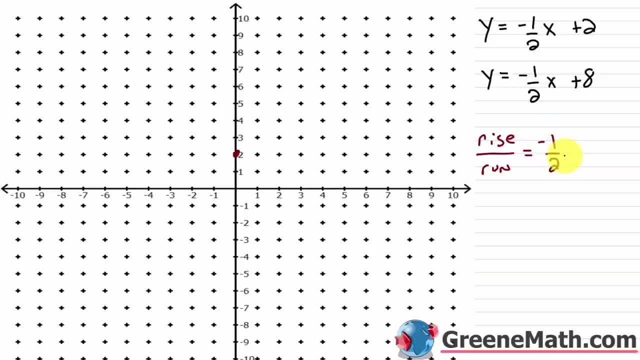 So this equals negative 1 over 2 or you could put 1 over negative 2 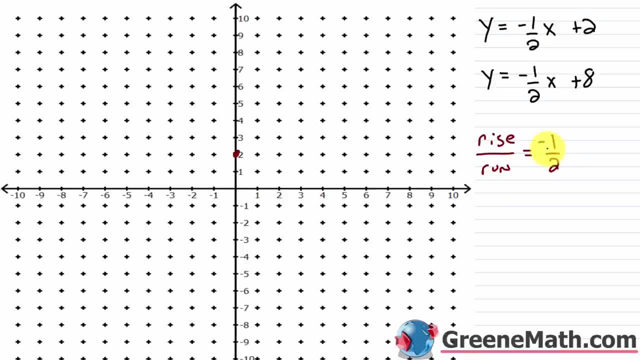 Doesn't really matter how you kind of think about that So if my rise is negative 1 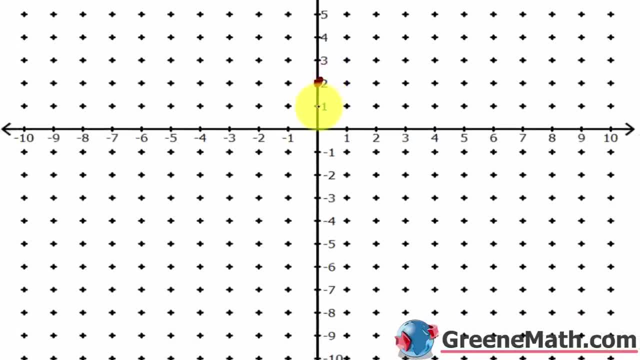 that means I fall 1 and if my run is 2, positive 2 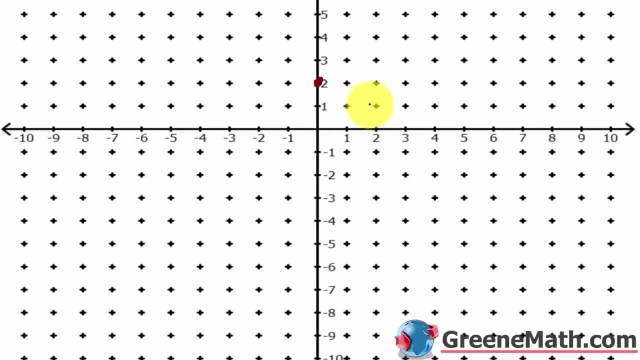 that means I go over to the right 2 So 1, 2. So there's my next point 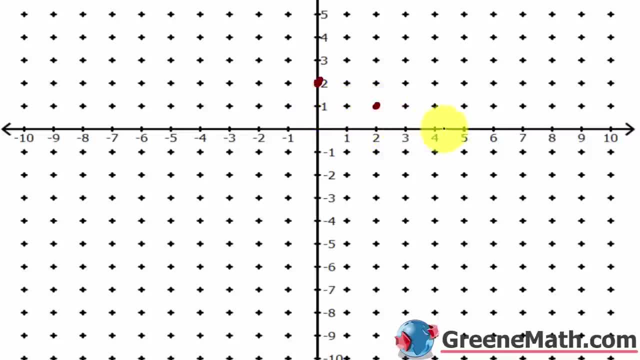 Down 1 over 1, 2 There's my next point 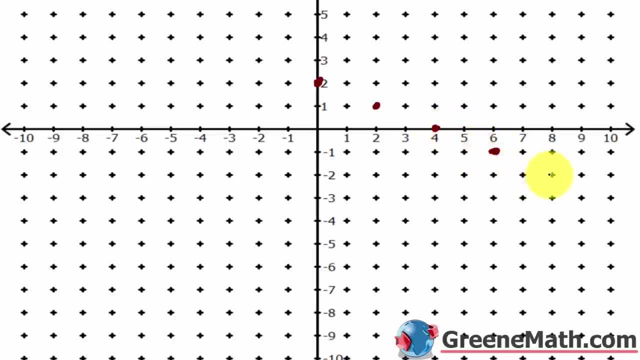 Down 1 over 1, 2 There's my next point 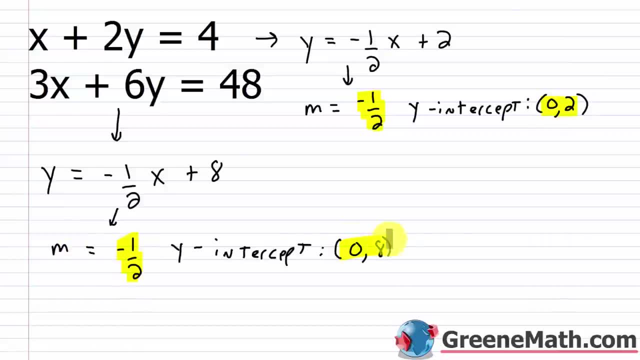 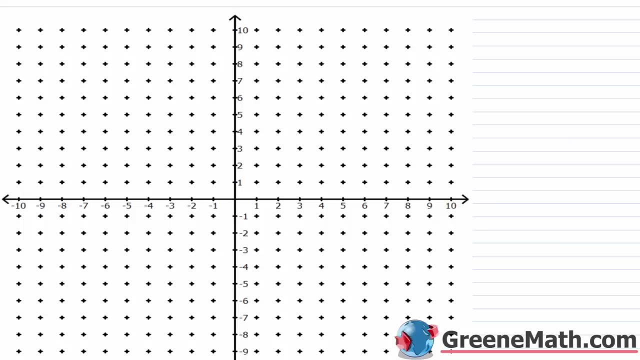 same slope, different y intercepts, different y intercepts. we know that we have parallel lines, so these lines are parallel. so one thing i want to show you really quickly is what this visually looks like using a coordinate plane. so remember, we had y equals negative one, half x plus two. 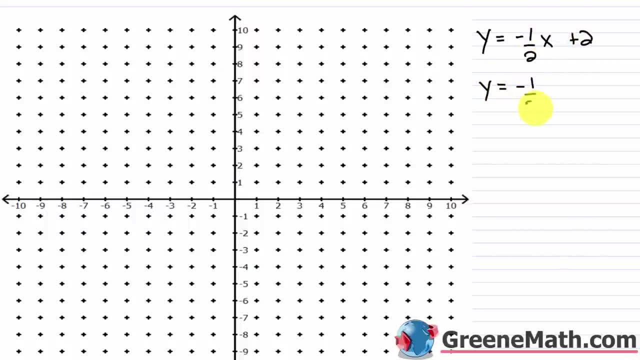 and we had y equals y equals negative one half x plus two, and we had y equals negative one half x plus two, negative one half x plus eight in slope intercept form. these are our two lines. now if we know a point on the line and the slope we can easily graph right. remember, we've kind of transcended the. 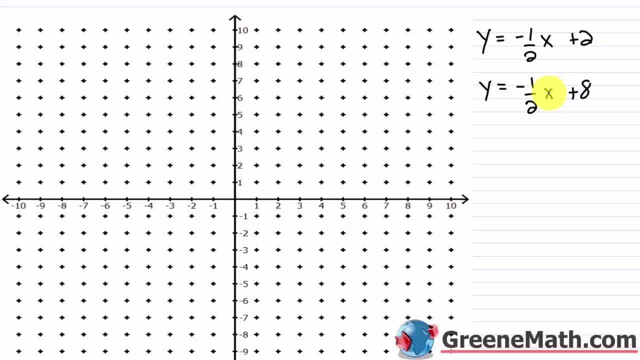 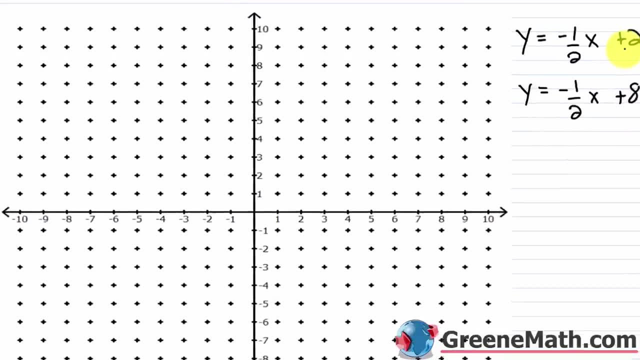 point where we have to go through and make ordered pairs and do all this stuff. we can graph really quickly now. so i know for this first one the y intercept occurs at zero comma two. so on the coordinate plane that's going to be right here and then my slope is negative. 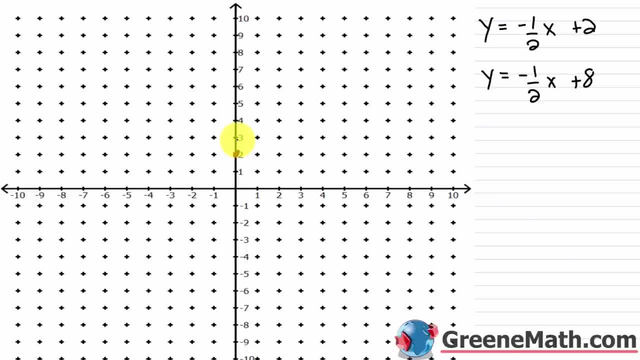 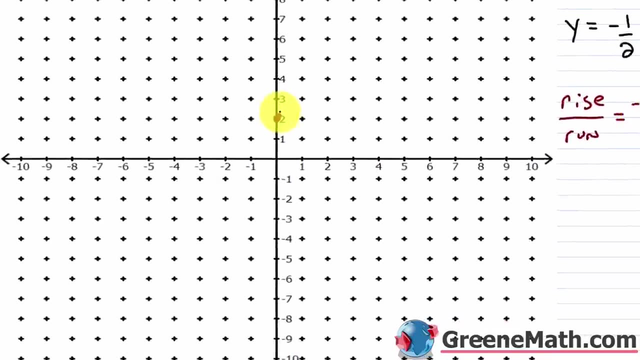 one half. so remember it's rise over run, it's rise over run. so this equals negative one over two, or you could put one over negative two, doesn't really matter how you kind of think about that. so if my rise is negative one, that means i fall one, and if my run is two, positive two, that means i go over to. 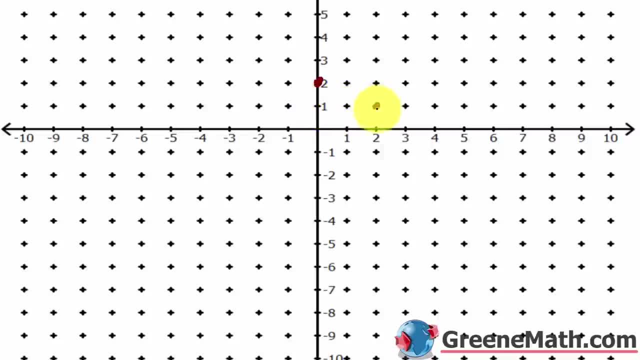 the right: two, so one, two. so there's my next point down: one over one, two. there's my next point down. one over one, two. there's my next point down: one over one, two. there's my next point. or, like I said, I could have also done one over negative two. so if I 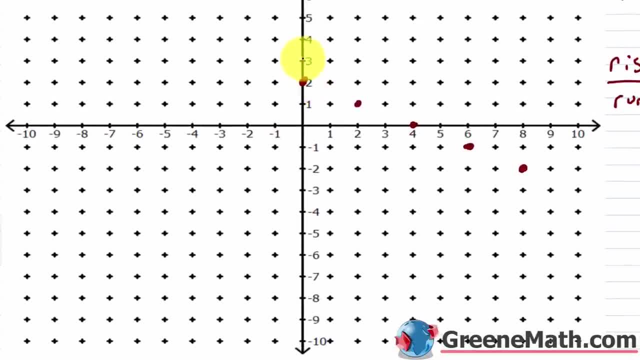 started here, I would rise one, and if I have negative two in the denominator, that means I go to the left two. so I go one, two to the left up, one to the left, one, two. and obviously you don't need all these points to make a line, but I like. 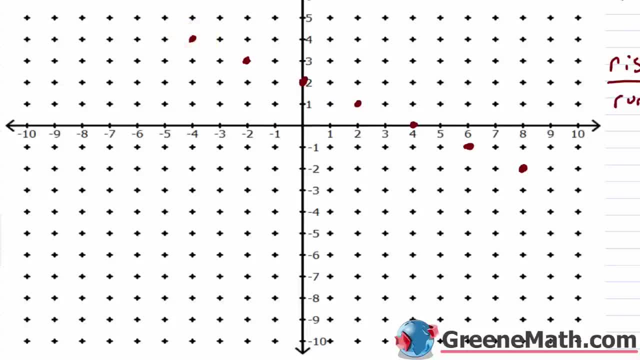 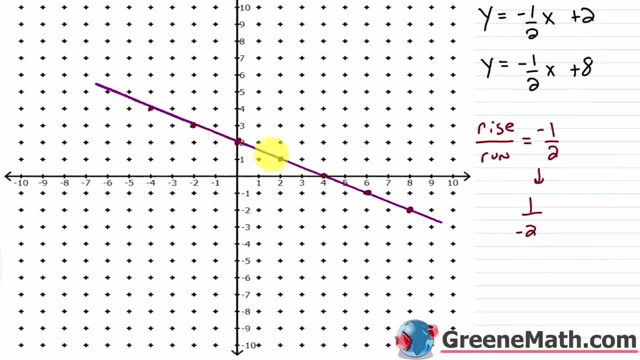 to kind of do that when we're in our first stages, just to kind of get our brain used to graphing a line this way. okay, all right for the next one. here we have y equals negative one half, X plus eight. and again we know a point on this line: it's at zero comma eight. so that's. 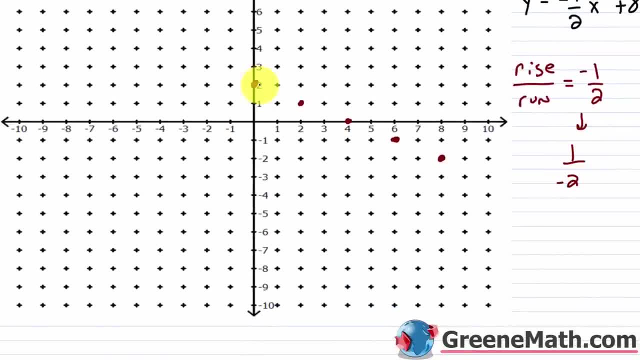 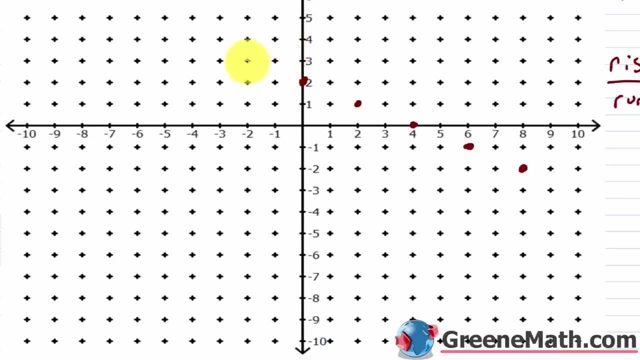 And I could have also done 1 over negative 2 So if I started here I would rise 1 and if I had negative 2 in the denominator that means I go to the left 2 so I go 1, 2 to the left Up 1 to the left 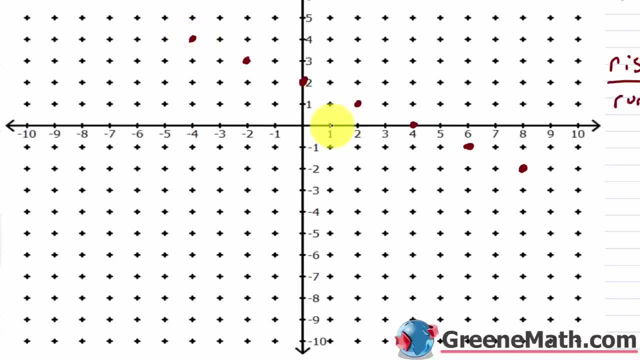 and obviously you don't need all these points to make a line but I like to do that when we're in our first stages just to kind of get our brain used to graphing a line this way 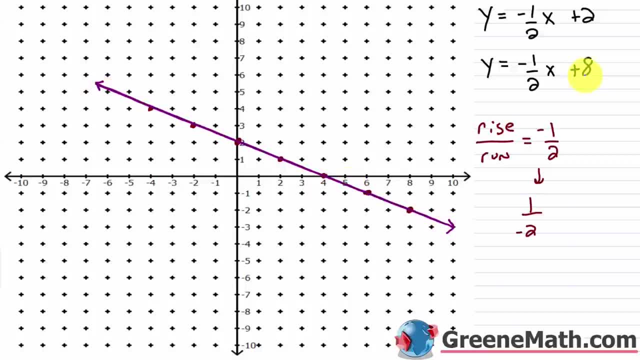 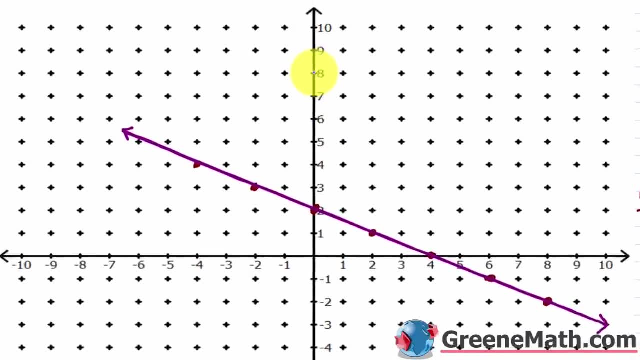 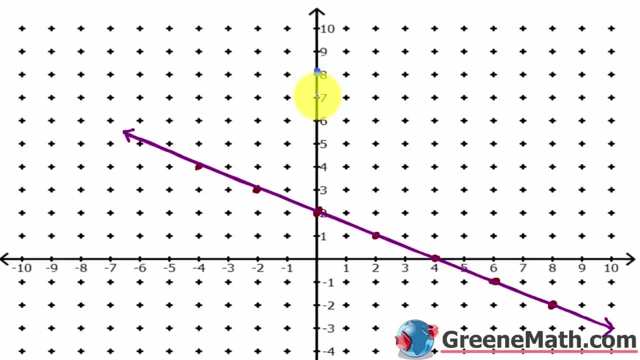 Alright, for the next one here we have y equals negative 1 half x plus 8, and again we know a point on this line, it's at 0 comma 8, so that's going to be right here. And then to graph it, again we just use that slope negative 1 half, so I can fall 1 and go to the right 2, fall 1 go to the right 2, fall 1 go to the right 2, fall 1 go to the right 2, and I'll go ahead and stop there. 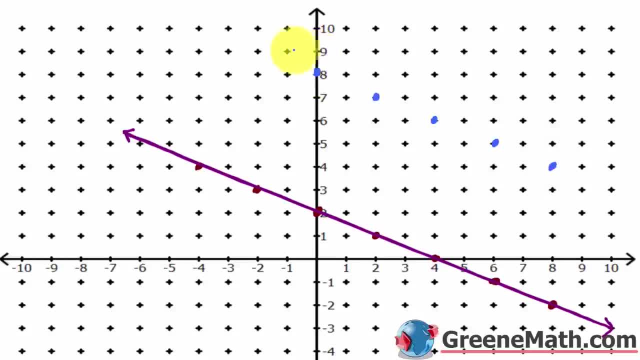 Or another thing I could do, again I could use this, I could go up 1 and to the left 2. 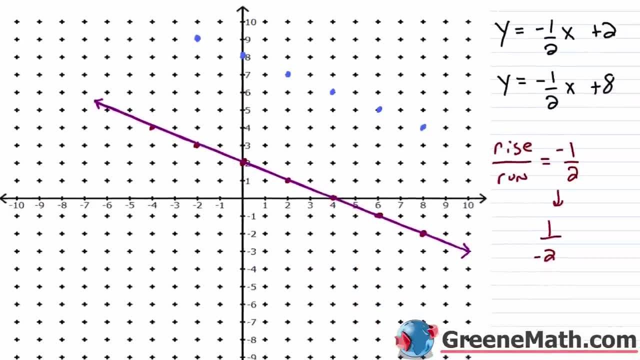 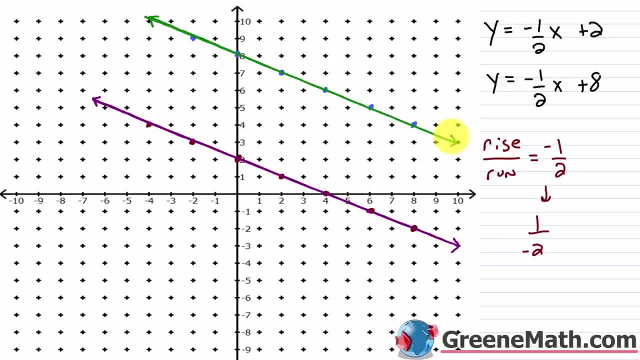 So let's go ahead and graph this. Some arrows in, and let me kind of erase this part real quick. 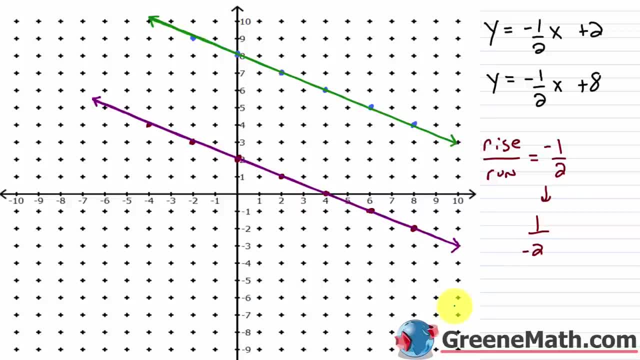 Alright so it's not perfect and no graph that you ever freehand draw will be, I mean some of them are pretty good, but you know if you were to put these equations in on a computer graphing program. You could really see. But even just looking at this simple hand drawing here, you can tell that these lines pretty much look the same, right, they have the same steepness or the same slope. What's really different about them is that they are on different parts of your coordinate plane, right, they have different y intercepts. This one has a y intercept that's at 0 comma 2. 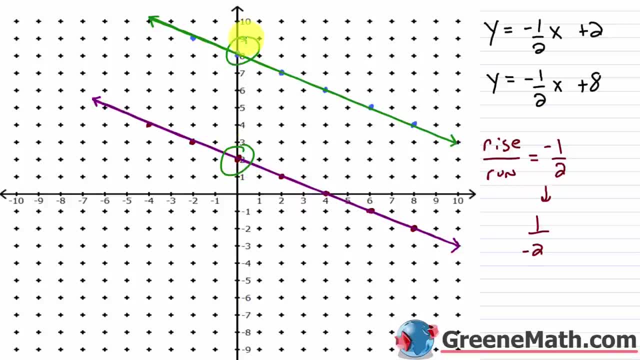 This one has a y intercept that's at 0 comma 8. But if you were to extend these lines out indefinitely in each direction, because they're parallel to each other. 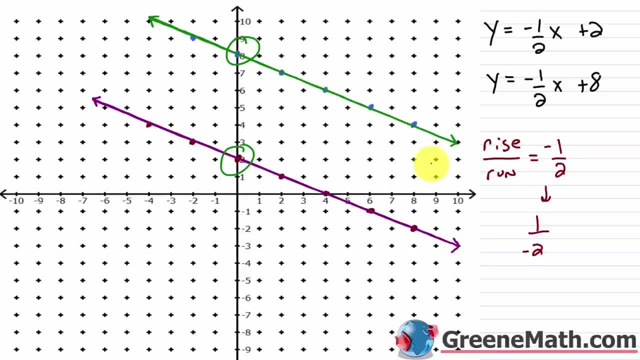 They will never ever ever touch. So that's what we're trying to get across here. 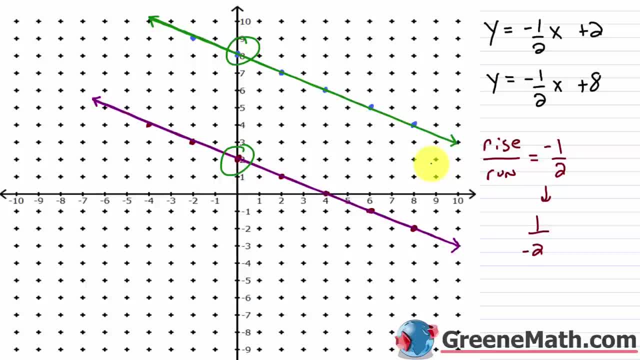 So again, two non-vertical parallel lines will look like this. They have the same slope, but different y intercepts. 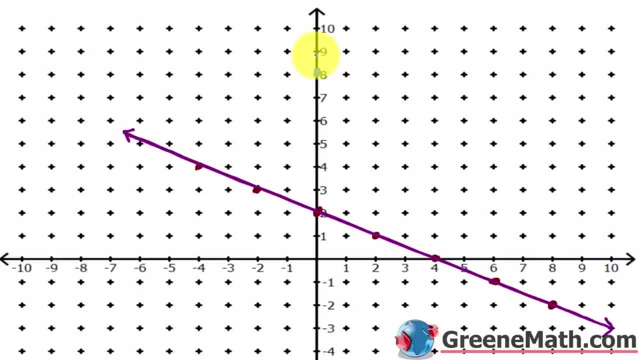 gonna be right here, and then to graph it again, we just use that slope negative one half, so I can fall one and go to the right to fall one, go to the right two, fall one, go to the right to fall one, go to the right two, and I'll go ahead and 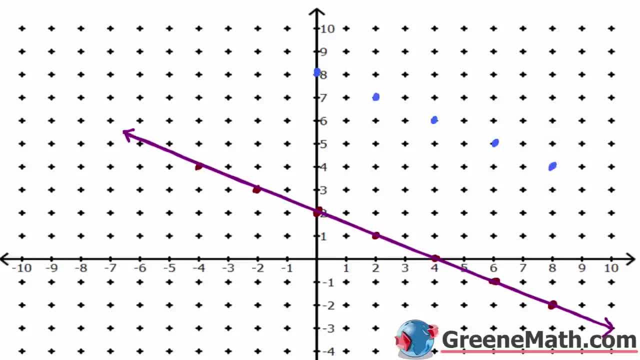 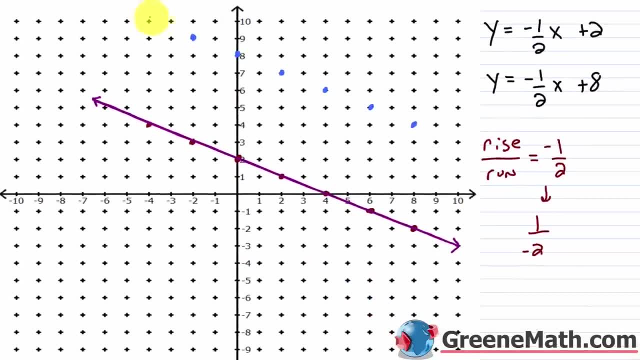 stop there, or another thing I could do again. I could use this. I could go up one into the left. two, let's go ahead and graph this, some arrows in, and let me kind of erase this part real quick. all right, so it's not perfect and no graph. 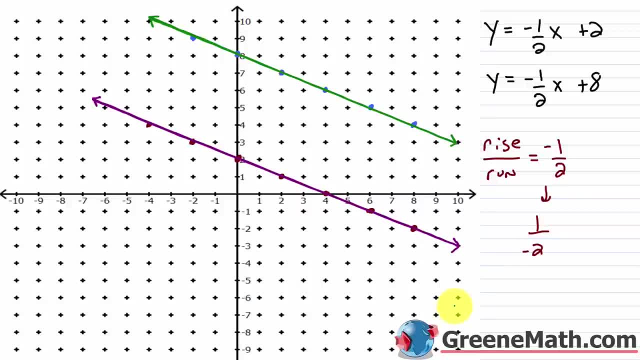 that you ever freehand draw will be. I mean, some of them are pretty good, but you know, if you were to put these equations in on you know a computer graphing program you can really see. but even just looking at this simple hand drawing here you can tell that these lines pretty much look the same right. 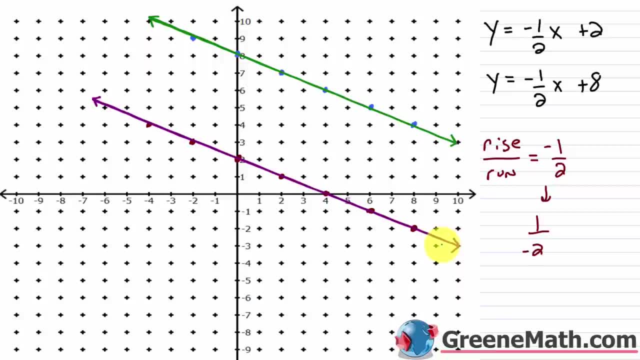 they have the same steepness or the same slope. what's really different about them is that they are on different parts of your coordinate plane. right, they have different y intercepts. this one has a y intercept that's at zero comma two. this one has a y intercept that it's at zero, comma three. phenomena: these lines 62 plus and dedim, you know a Venus bogey we weren't right into. 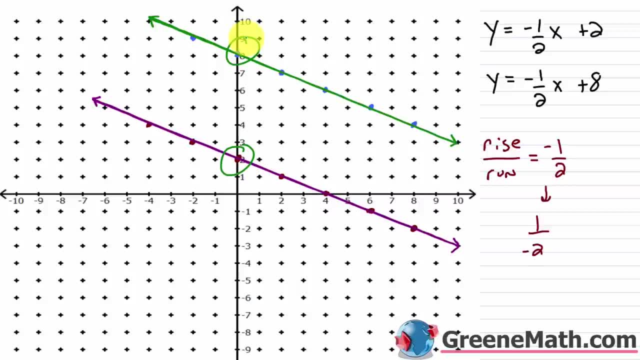 inner seventh square was charged, taking up frequency. it's on this first Korean Willl, comma 8.. But if you were to extend these lines out indefinitely in each direction, because they're parallel to each other, they will never, ever, ever touch. Okay, so that's what we're trying to get. 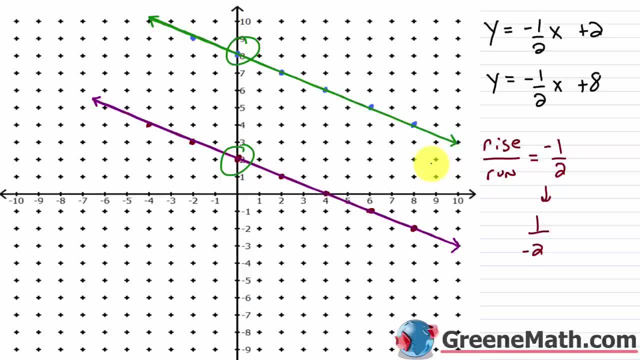 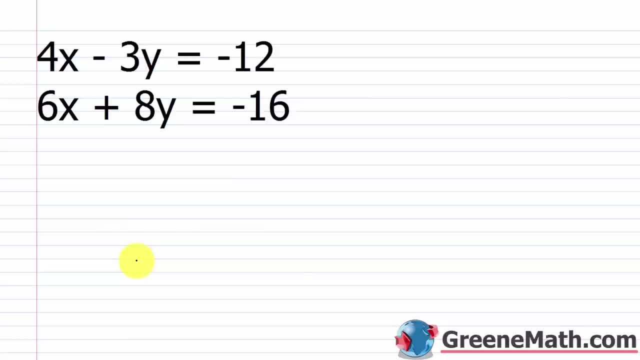 across here. So again, two non-vertical parallel lines will look like this: They have the same slope but different y-intercepts. All right, let's take a look at another one. We have 4x minus 3y equals negative 12, and we have 6x plus 8y equals negative 16.. Okay, so again I'm going to solve each for y. 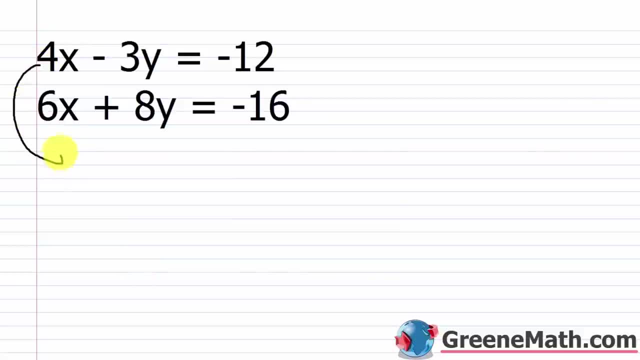 and I'm going to do this a little quicker this time. So we'll move this over here and say: okay, I have 4x minus 3y equals negative 12. Subtract 4x away from each side of the equation, so that's. 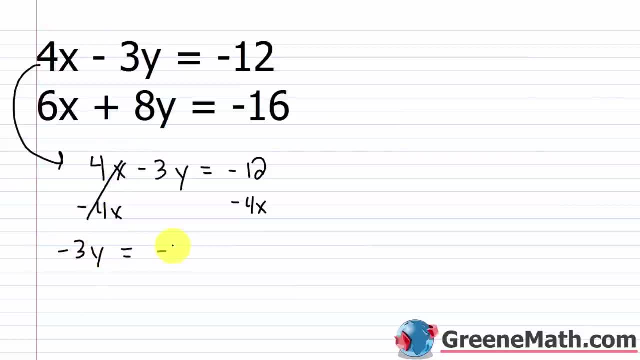 gone I'd have a negative 3y is equal to negative 4x minus 12.. All right, so the next thing I want to do is divide both sides of the equation. So I'm going to divide both sides of the equation. and I'm going to divide both sides of the equation. So I'm going to divide both sides of the equation. 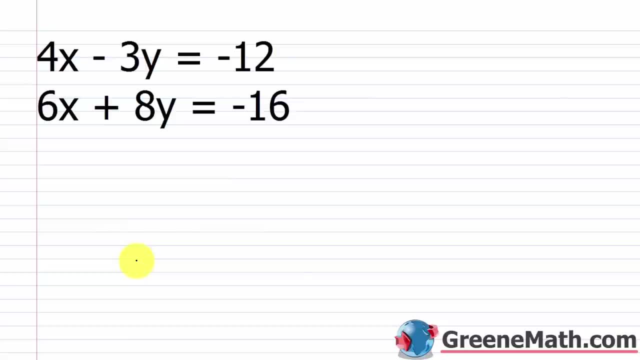 Alright let's take a look at another one. We have 4x minus 3y equals negative 12, and we have 6x plus 8y equals negative 16. 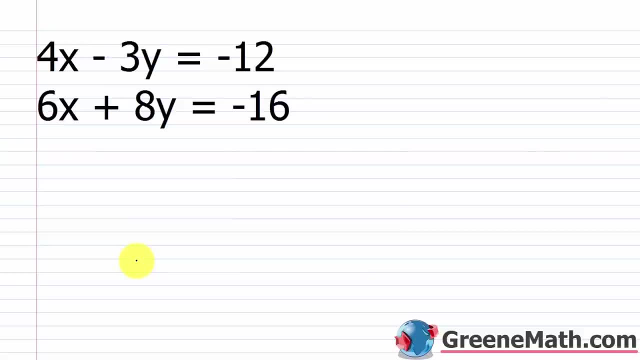 Okay so again I'm going to solve each for y, and I'm going to do this a little quicker this time. 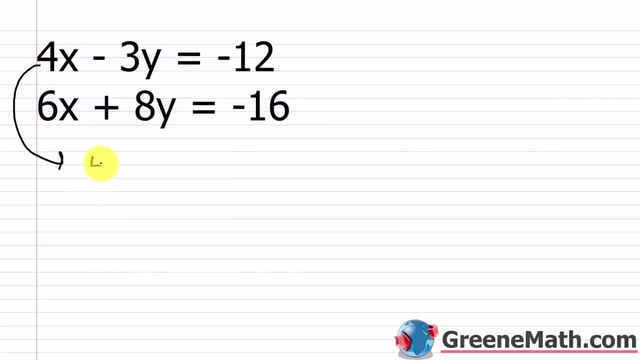 So we'll move this over here and say okay. I have 4x minus 3y equals negative 12. 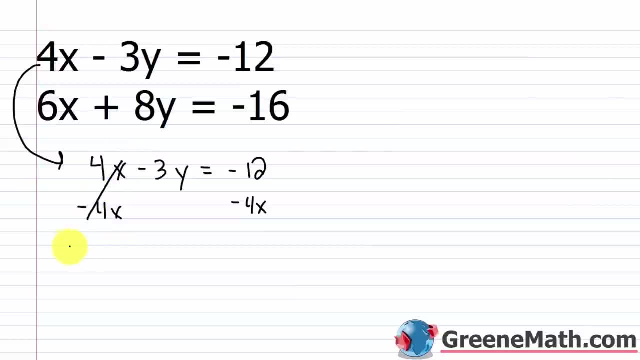 Subtract 4x away from each side of the equation. So that's gone. 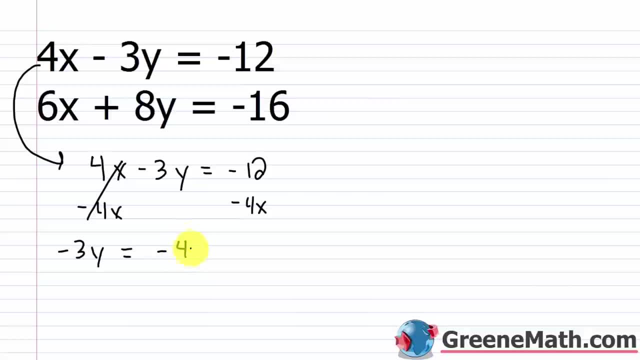 I'd have negative 3y is equal to negative 4x minus 12. Alright so the next thing I want to do is divide both sides of the equation by negative 3, the coefficient of y. 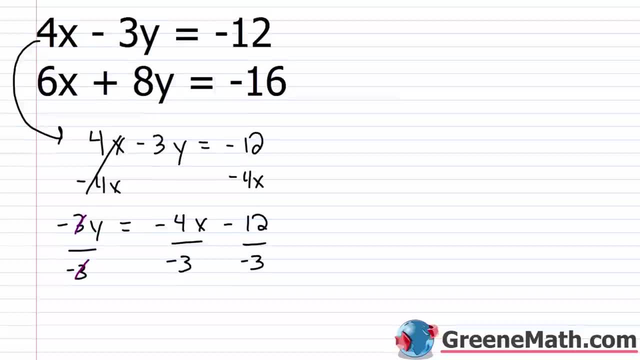 So that is going to cancel with that, and I'll have y by itself, and this is equal to negative 4 over negative 3 is just 4 over 3. 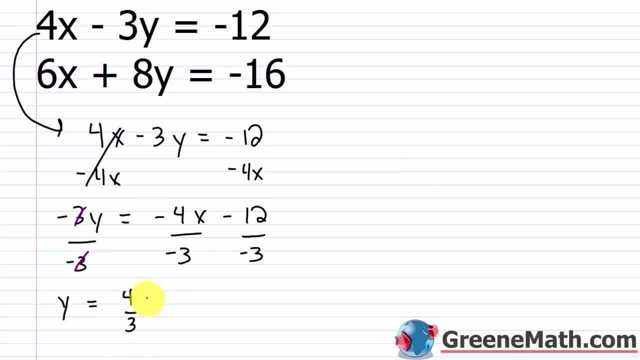 Or 4 thirds, right the negatives would cancel, times x, and then the negatives would cancel again. 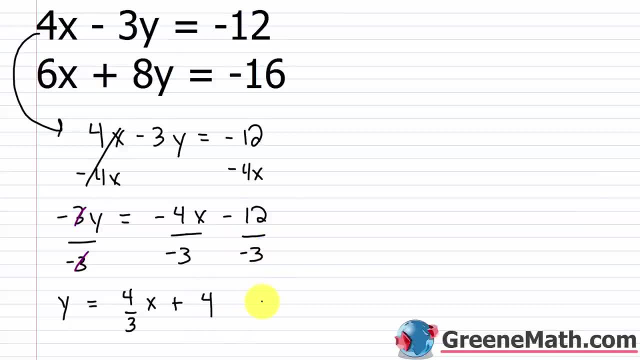 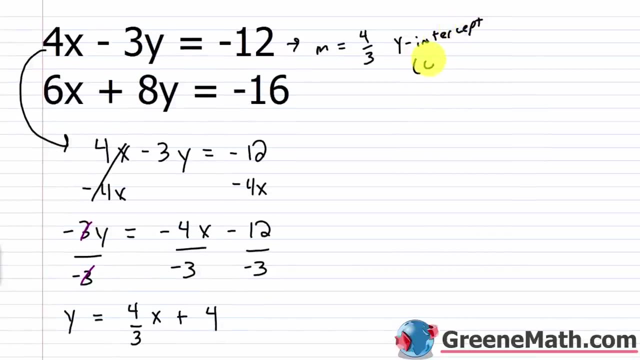 So plus 12 over 3 is 4. So I know for this one that the slope, which is m, is equal to 4 thirds, and that the y intercept, the y intercept, is going to occur at . Alright for the next one. Again. 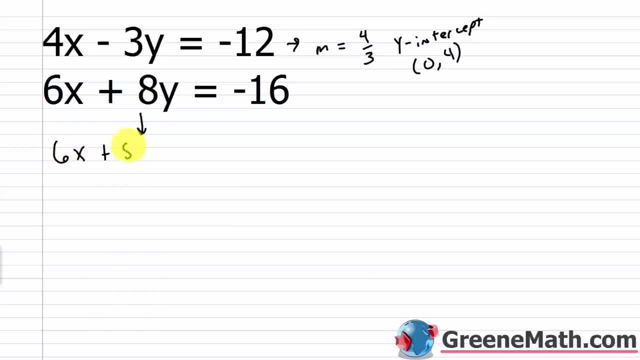 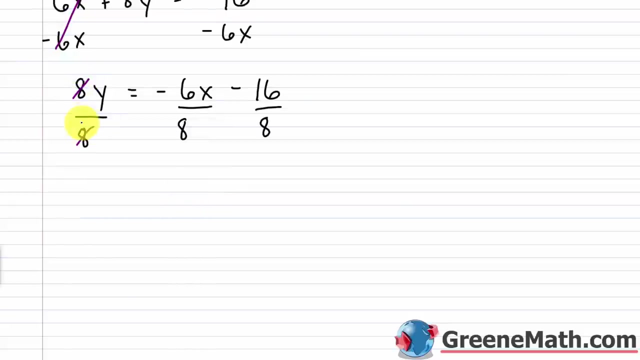 I'm trying to solve this for y. So 6x plus 8y equals negative 16. I'm going to subtract 6x away from each side of the equation. So this is going to cancel, and I'm going to have 8y is equal to negative 6x minus 16. Divide each side by 8. So I'm going to cancel this 8 with this 8, and I'm going to have y is equal to, so 6 divided by 2 would be 3. 8 divided by 2 would be 4. So this would be negative 3 fourths times x, and then minus, 16 over 8 is 2. 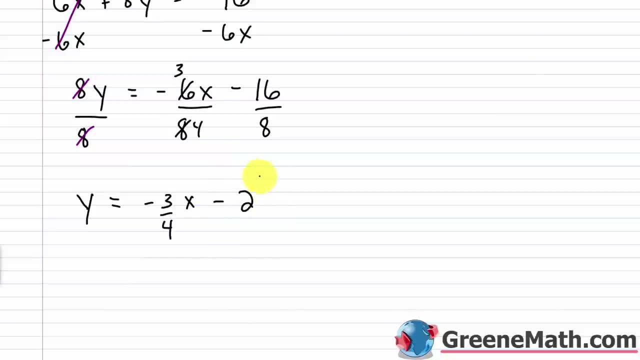 So my slope here is negative 3 fourths. My y intercept occurs at . 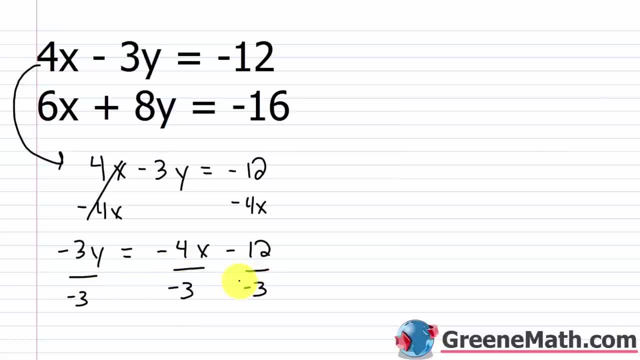 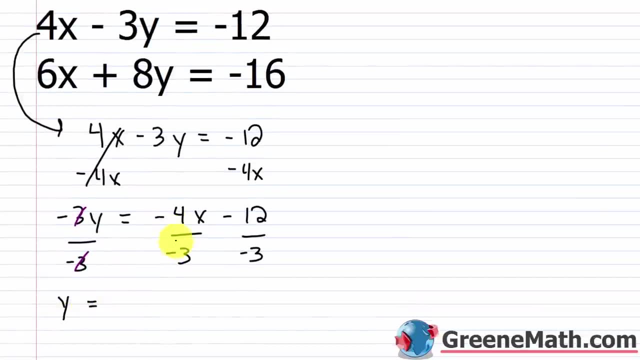 by negative 3 the coefficient of y. so that is going to cancel with that and I'll have y by itself and this is equal to negative 4 over negative 3 is just 4 over 3 or 4 thirds. right, the negatives would cancel times x and then the negatives would cancel again. so plus 12 over 3 is 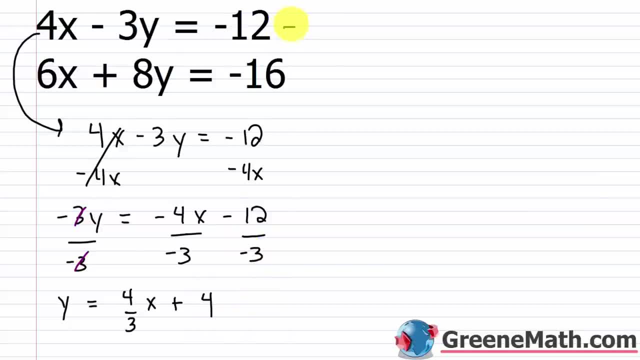 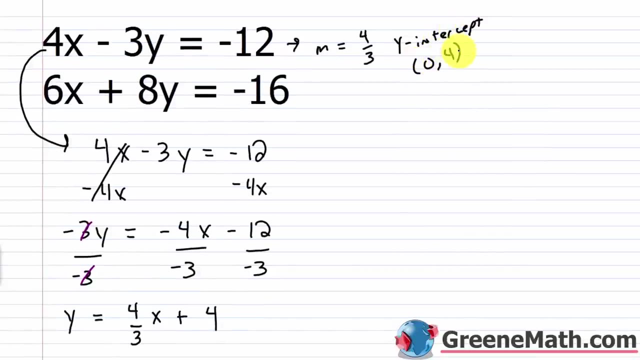 4. so I know for this one that the slope which is M is equal to 4 thirds and at the y-intercept the y-intercept is going to occur at zero comma four. all right, for the next one. again, I'm trying to solve this. for why? so? 6x plus 8y equals negative 16. I'm gonna subtract 6x away from. each side of the square root of 4. so I can just write that down over here. but you actually heat out and put this right. so negative 4 over 3 taken basically goes out of the four tenths as 1 over each of the ela, as sum of the fouringthe first ribs equal à 2. and this is where 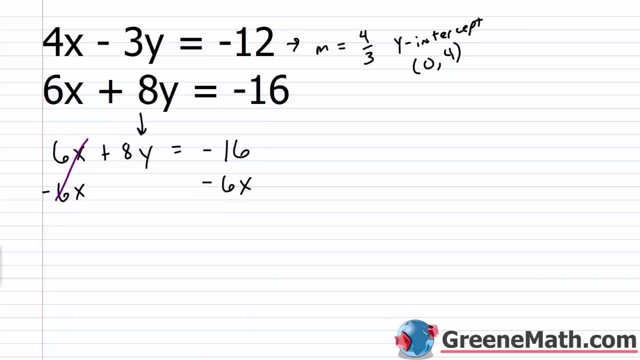 I take 3x divided into 1, to make that square root plus 3. we would calculate here. so these of the equation. So this is going to cancel And I'm going to have. 8y is equal to negative 6x minus. 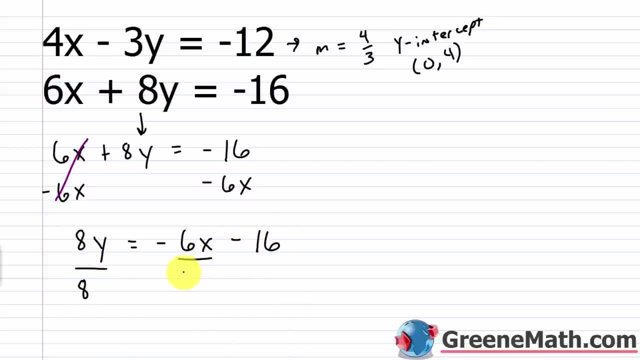 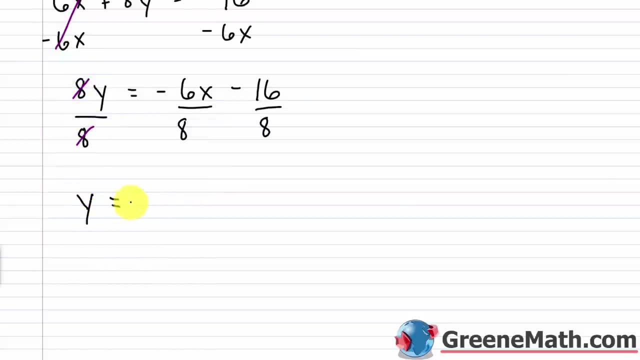 16.. Divide each side by 8.. So I'm going to cancel this 8 with this 8. And I'm going to have: y is equal to, so 6 divided by 2 would be 3.. 8 divided by 2 would be 4.. So this would be negative 3 fourths. 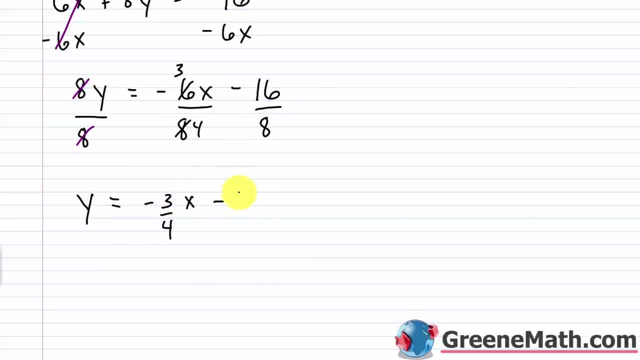 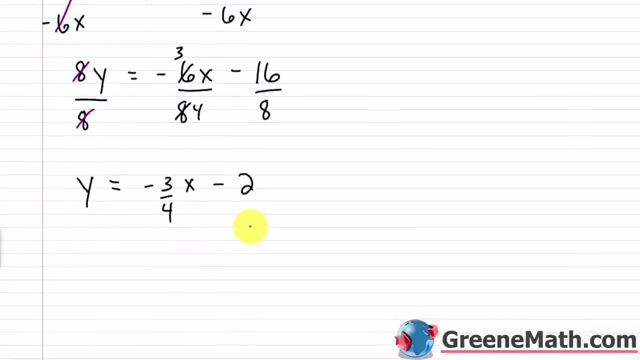 times x, And then minus 16 over 8 is 2.. So my slope here is negative 3 fourths. My y intercept occurs at 0 comma, negative 2.. So m is equal to negative 3 fourths And again y intercept. 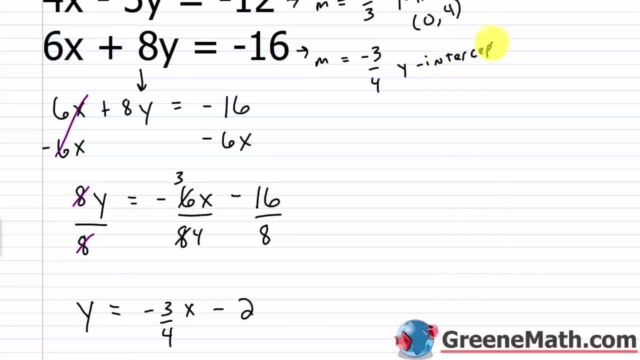 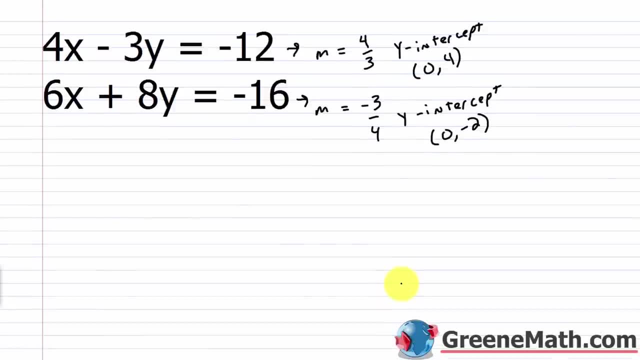 is at 0 comma negative 2.. So kind of the first question you're going to ask yourself here is: are these lines parallel? Well, you would be talking about all the different 내려ving to take into account, And I'm going 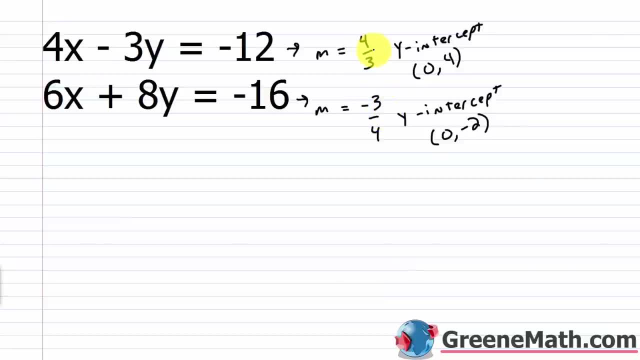 into a little more detail on the differences between the two And I'm going to walk through. you see that the slopes are clearly different numbers. right, This is four-thirds. this is negative three-fourths. If they're different values, you don't have parallel lines Now. 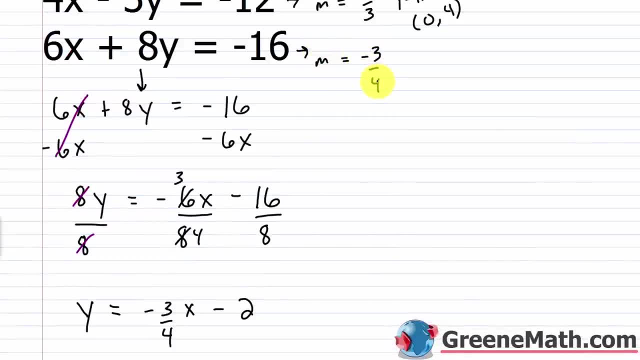 So m is equal to negative 3 fourths, and again y intercept is at . So it kind of looks like this. I'm going to write this down. I'm going to write this down. 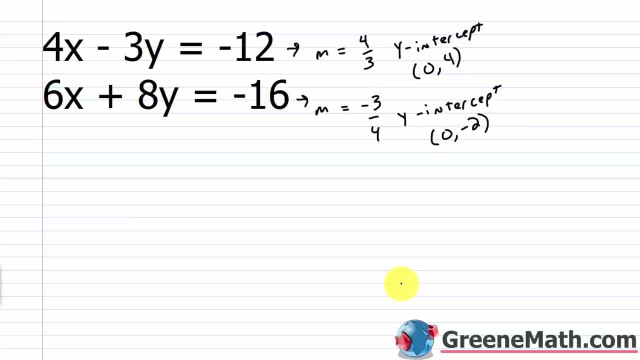 So kind of the first question you're going to ask yourself here is, are these lines parallel? Well, you see that the slopes are clearly different numbers, right? This is 4 thirds. This is negative 3 fourths. 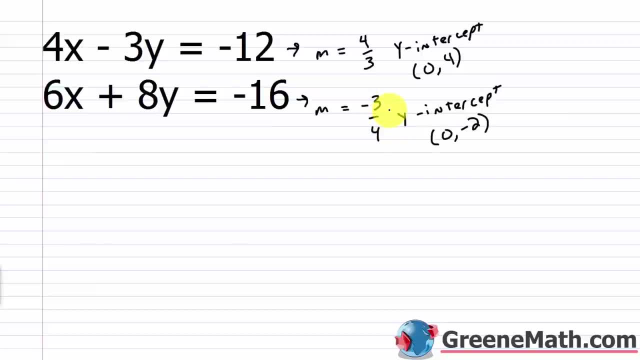 If they're different values, you don't have parallel lines. Now the next thing you would ask yourself is, are these lines perpendicular? Well, perpendicular lines have a property that tells us that the product of the slopes would be negative 1. So in other words, if I took 4 thirds. Which is the slope for this equation here, and I multiplied it by negative 3 fourths, which is the slope for this equation here, I should get negative 1 if these two lines are perpendicular. 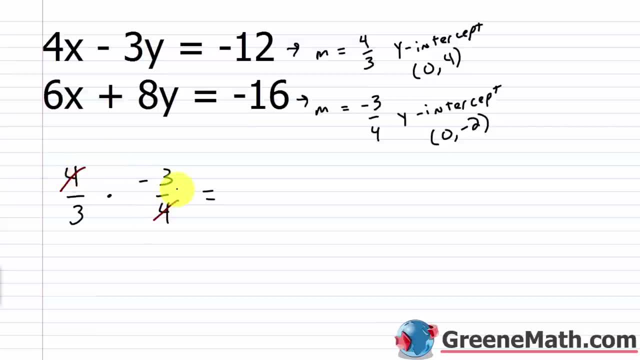 So you can see that you would, right? Because this 4 would cancel with this 4, 4 over 4 is 1. 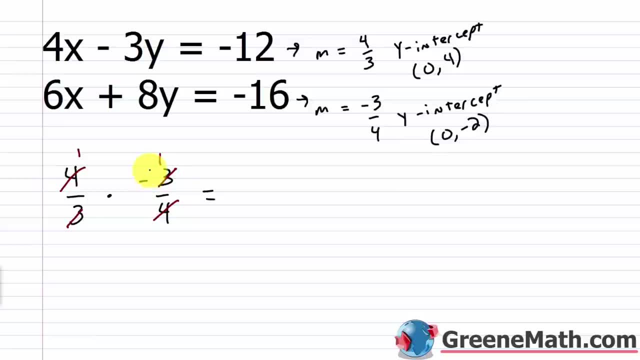 This 3 would cancel with this 3, 3 over 3 is 1, but I'm left with this negative here, right? 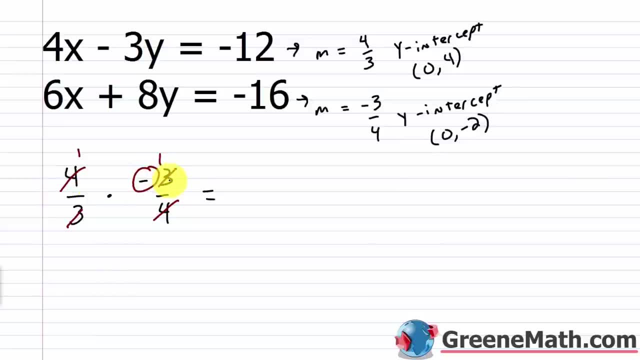 So I'd end up with 1 times negative 1, or just really everything canceling except for negative 1. And that would be my solution here, right? 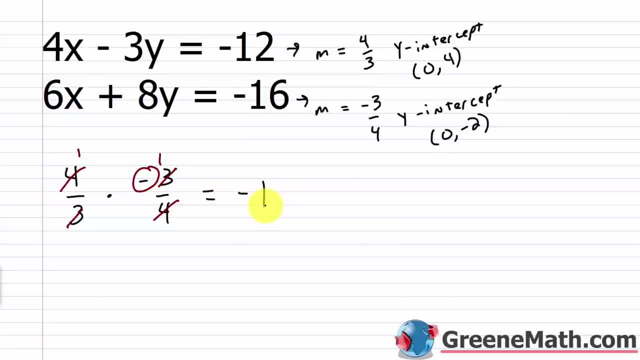 The product of the two slopes would in fact be negative 1. So we do have perpendicular lines. 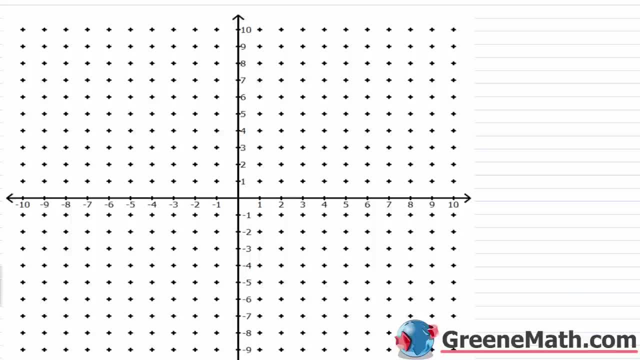 And again, to kind of look at this on a coordinate plane, let's take a look at our two equations in slope intercept form. 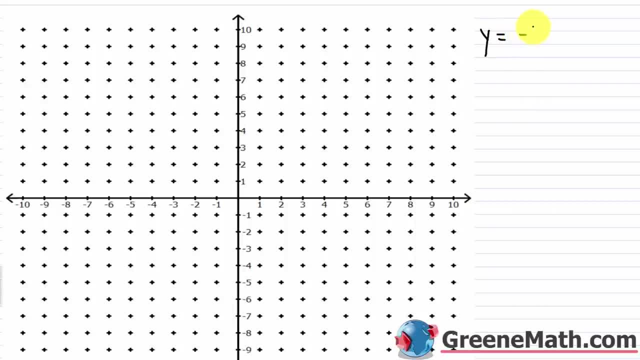 Again, we had y was equal to negative 3 fourths x. Minus 2. 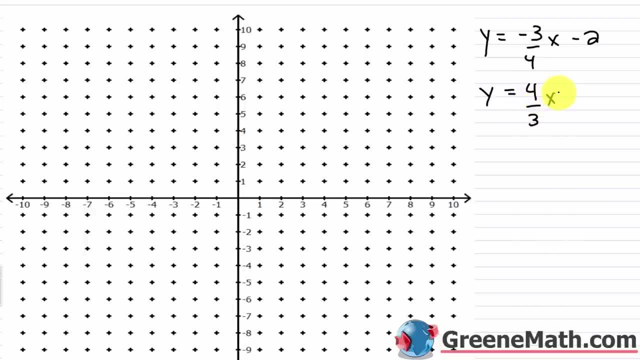 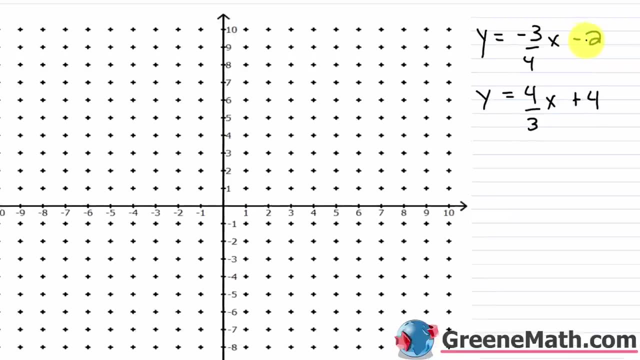 We also had y was equal to 4 thirds x plus 4. So again, really, really easy to graph these. We know the slope and we know the y intercept. So we have a point on the line in the slope. So for the first one, the y intercept is going to occur at 0 comma negative 2. That's right there. 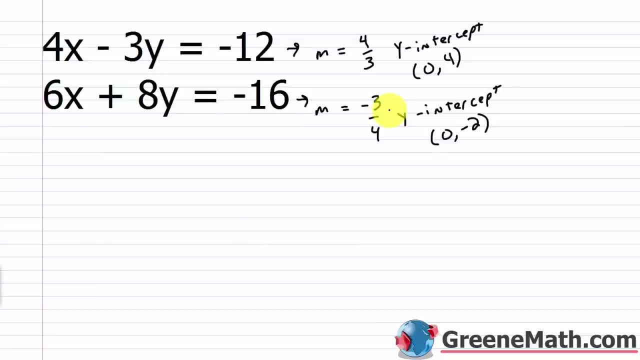 the next thing you would ask yourself is: are these lines perpendicular? Well, perpendicular lines have a property that tells us that the product of the slopes would be negative one. So, in other words, if I took four-thirds, which is the slope for this equation here? 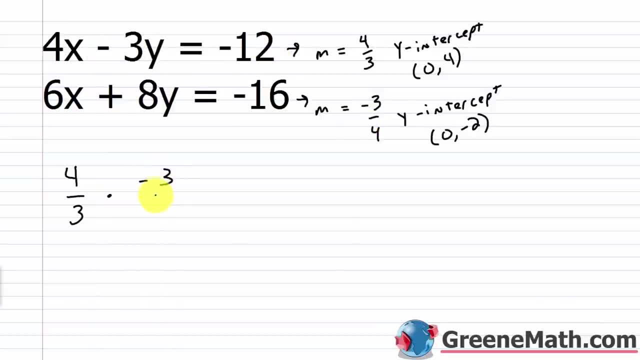 and I multiplied it by negative three-fourths, which is the slope for this equation. here I should get negative one if these two lines are perpendicular. So you can see that you would right, Because this four would cancel with this four. four over four is one. This three would. 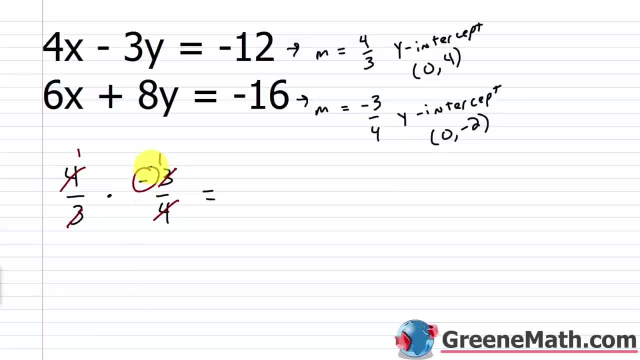 cancel with this three. three over three is one, but I'm left with this negative here, right? So I'd end up with one times negative one, or just really everything canceling except for negative one, and that would be my solution here. 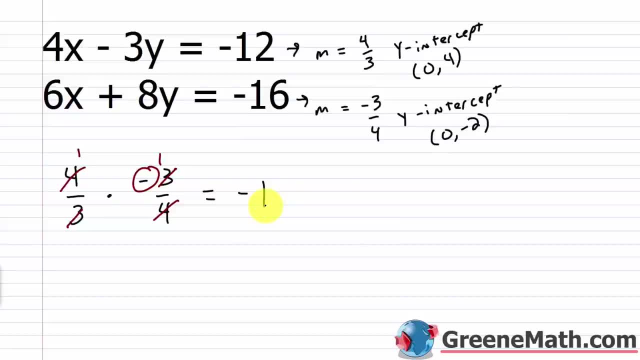 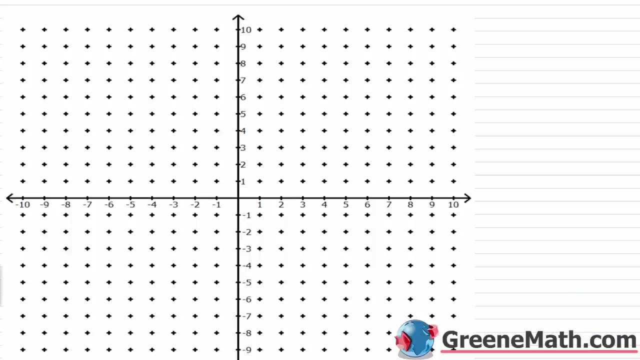 Right. The product of the two slopes would in fact be negative one. So we do have perpendicular lines And again, to kind of look at this on a coordinate plane, let's take a look at our two equations in slope-intercept form. Again, we had: y was equal to negative three-fourths x. 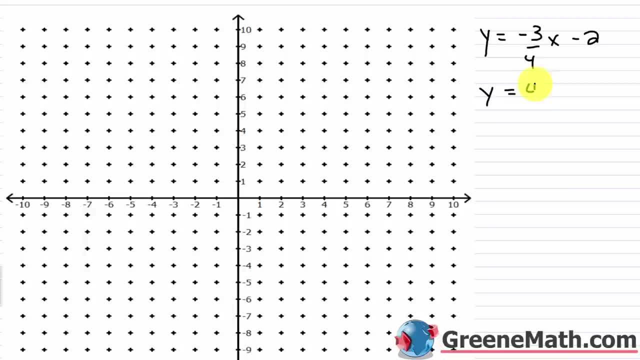 minus two. So we had y was equal to four-thirds x plus four. So again, really really easy to graph these. We know the slope and we know the y-intercept, So we have a point on the line. 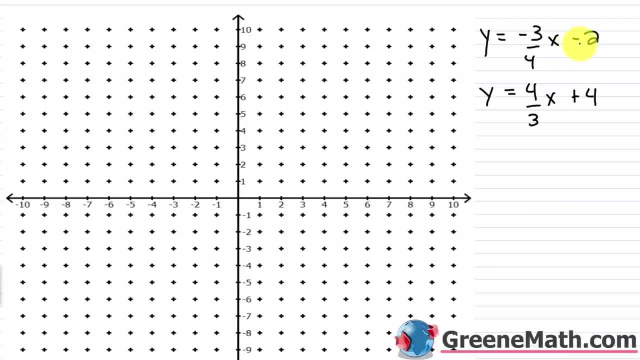 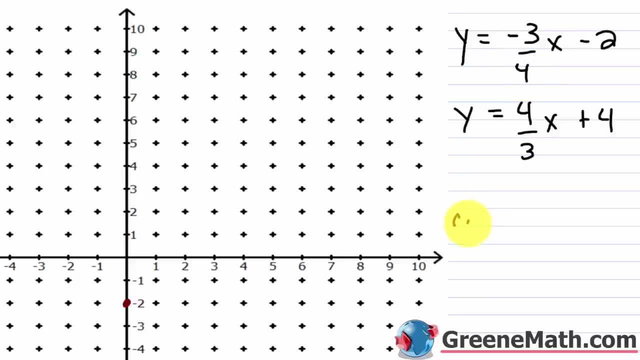 and the slope. So for the first one, the y-intercept is going to occur at zero comma negative two. That's right there. My slope is negative three-fourths. So again with rise over run, rise over run of negative three-fourths, or again you can think about: 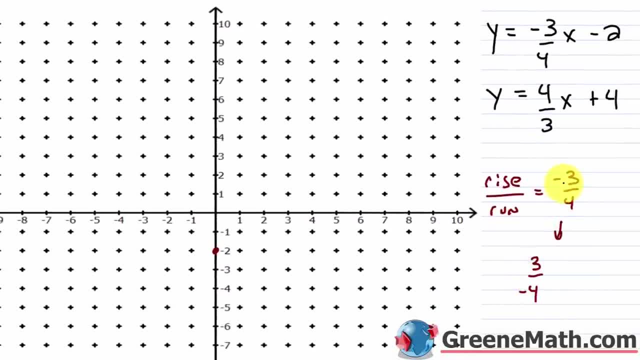 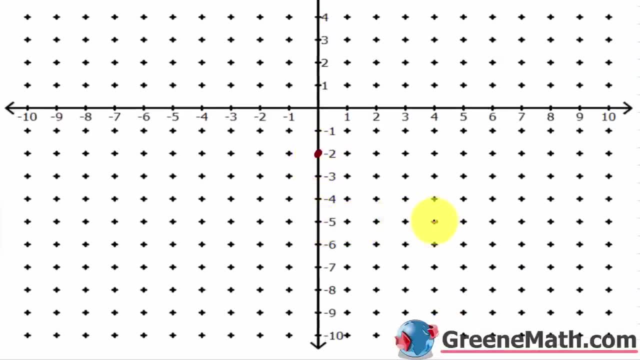 this as three over negative four Doesn't matter. In the first scenario I would fall three. I would fall one, two, three and I would run to the right. one, two, three, four. And I can make another point. but that's going to kind of go too far, So let me kind of. 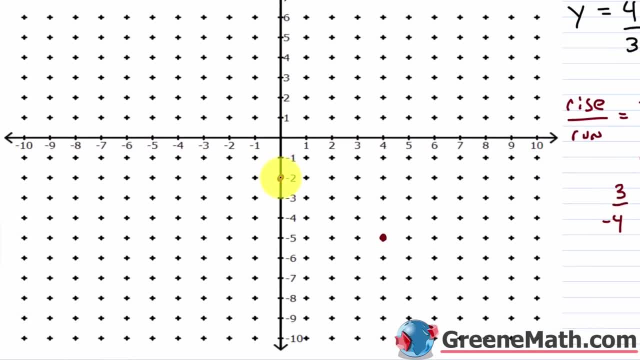 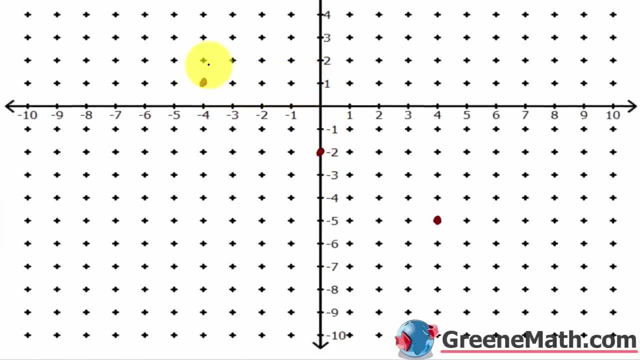 backtrack over here and let me use this now. Let me rise: three, One, two, three. Let me go to the left: four, One, two, three, four. So that's another point, And let me graph this real quick. 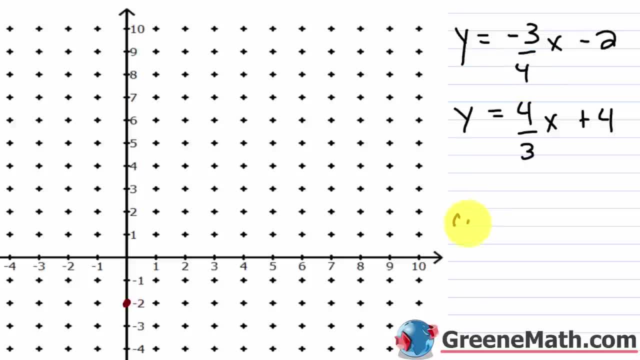 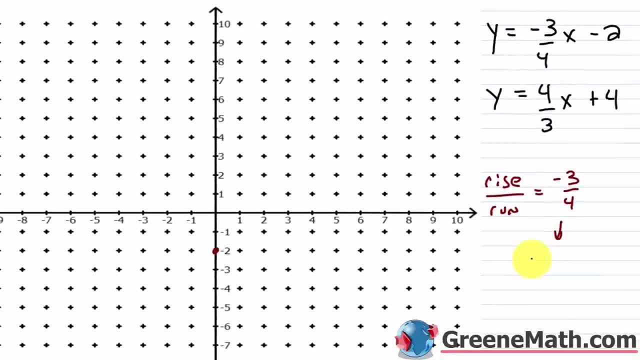 My slope is negative 3 fourths. So again, with rise over run. Rise over run. Overrun. Of negative 3 fourths. Or again, you can think about this as 3 over negative 4. Doesn't matter. In the first scenario, I would fall 3. I would fall 1, 2, 3. 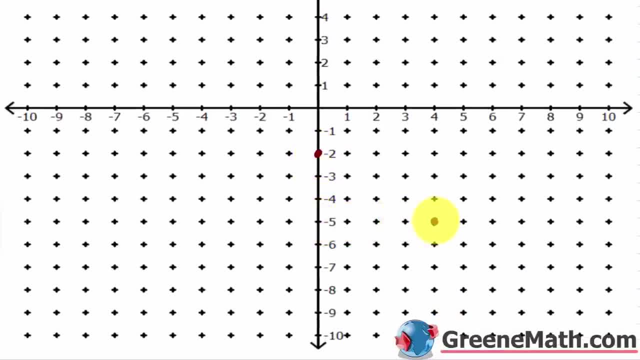 And I would run to the right 1, 2, 3, 4. And I can make another point. 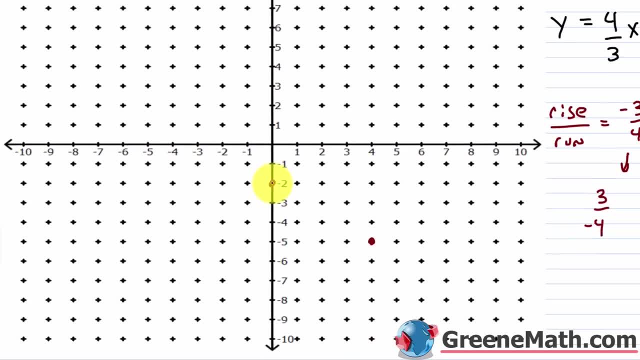 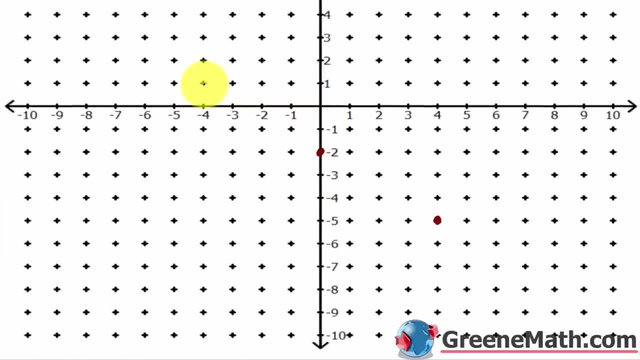 But that's going to kind of go too far. So let me kind of backtrack over here. And let me use this now. Let me rise 3, 1, 2, 3. Let me go to the left 4. 1, 2, 3, 4. 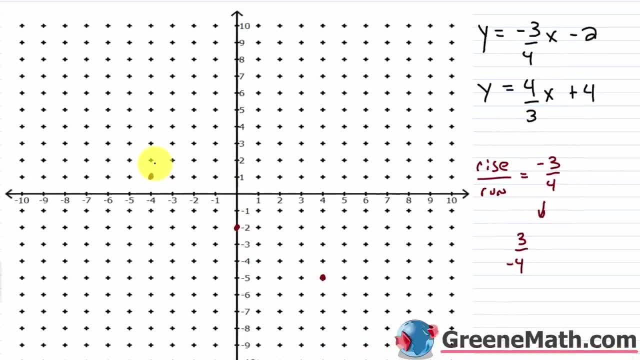 So that's another point. And let me graph this real quick. 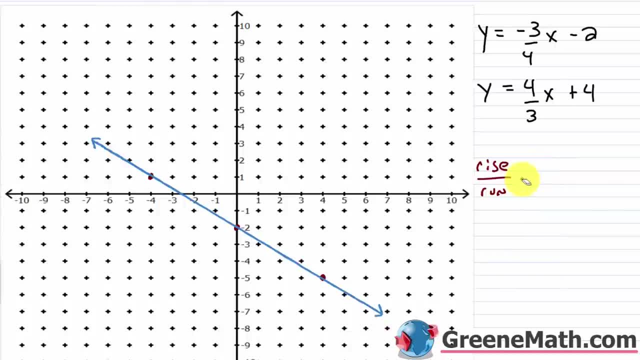 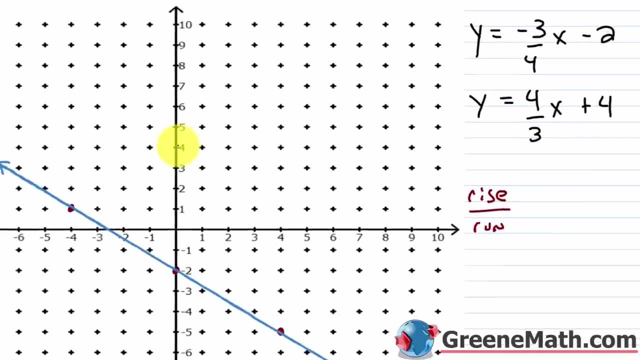 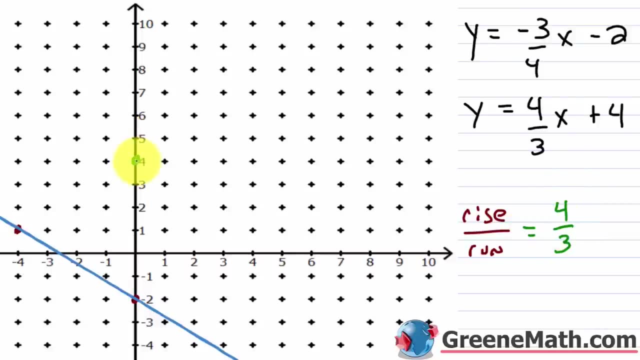 OK. And now for the next one, let me just erase this. We have y equals 4 thirds x plus 4. So the y intercept will occur at 0 comma 4. And that's going to be right here. And the slope is 4 thirds. So again, with rise over run, I can go up 4. So I can go up 1, 2, 3, 4. 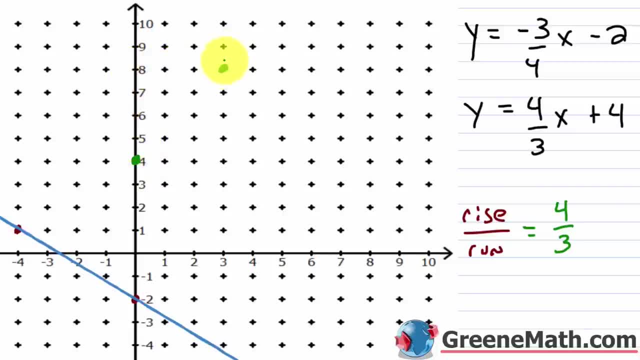 And to the right 1, 2, 3. And the other thing I can do, remember, negative over negative is also positive. So I can do negative 4 over negative 3. 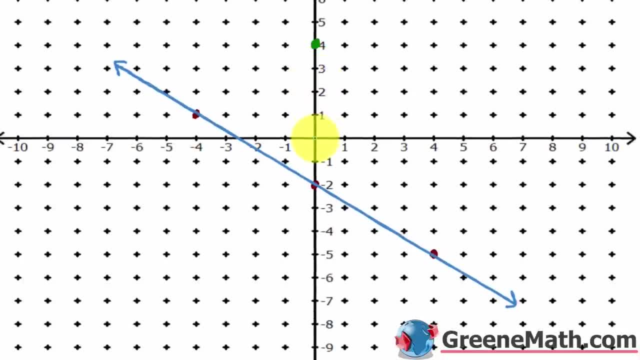 So I can fall 4. I can fall 1, 2, 3, 4. And go to the left 3. 1, 2, 3. So that's right there. And let me do one more point. 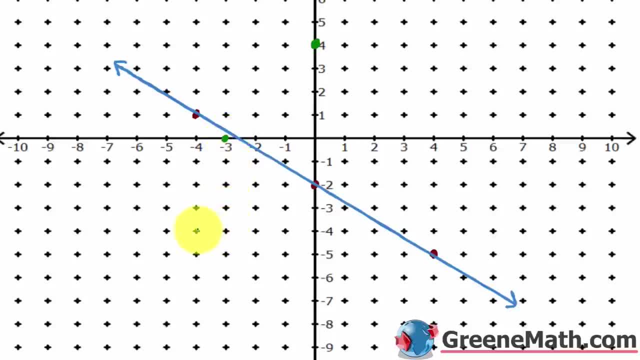 Fall 4, 1, 2, 3, 4 to the left 3. 1, 2, 3. OK. 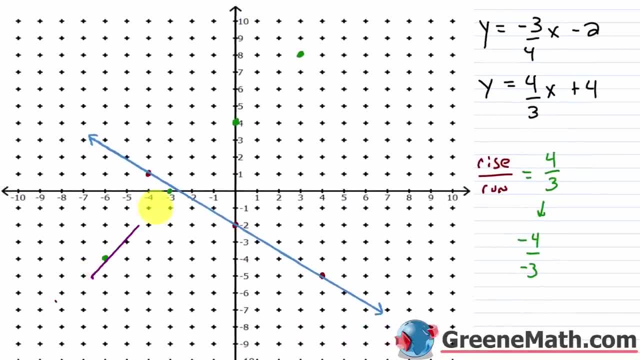 So let me graph this real quick. So one thing I want to draw your attention to, if you look at that point of intersection, you create a 90-degree angle there. This is a 90-degree angle. 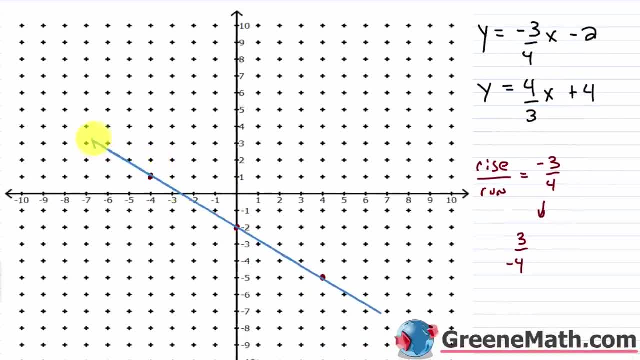 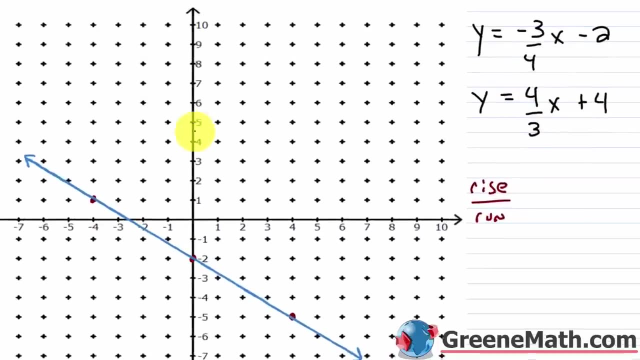 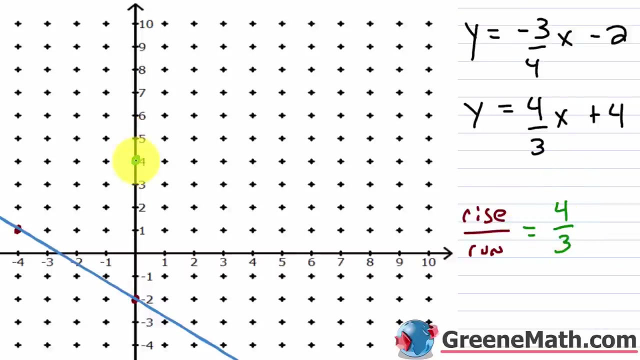 Okay, And now for the next one. let me just erase this. We have: y equals four-thirds, x plus four, So the y-intercept will occur at zero comma four, and that's going to be right here, And the slope is four-thirds. So, again, with rise over run, I can go up. 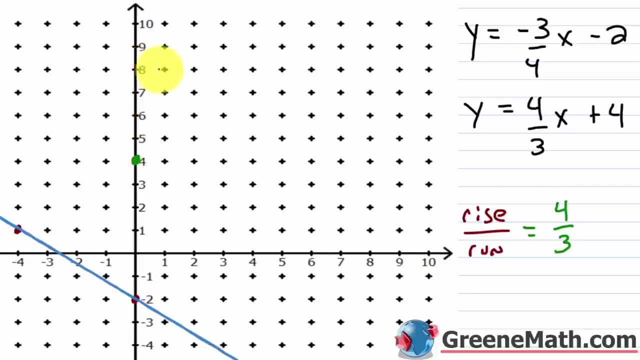 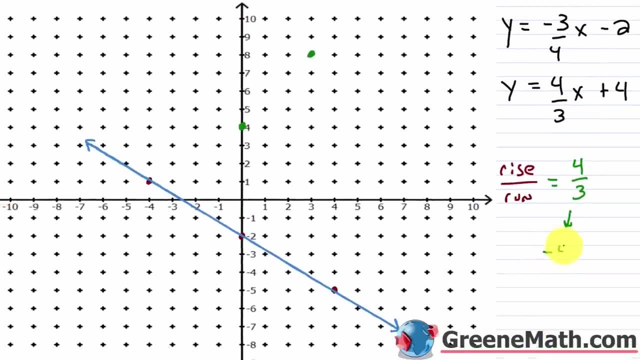 four. So I can go up one, two, three, four. and to the right, one, two, three. And the other thing I can do, remember, negative over negative is also positive, So I can do negative four over negative three, So I can fall four. I can fall one, two, three. 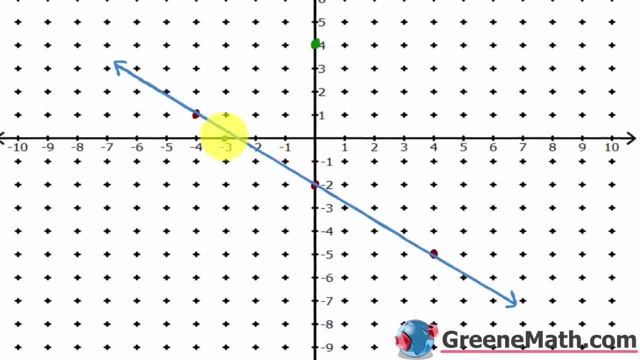 four and go to the left: three, One, two, three. So that's right there, And let me do one more point: Fall four, One, two, three. four. to the left: three, One, two, three. 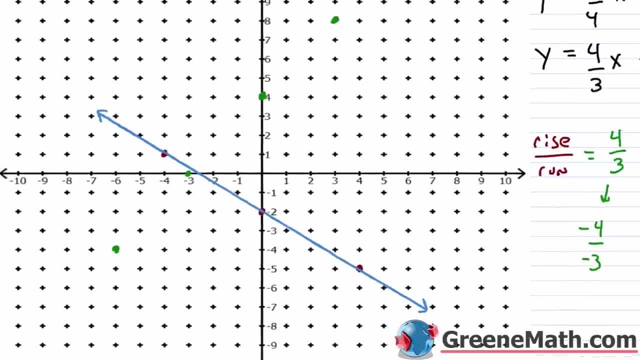 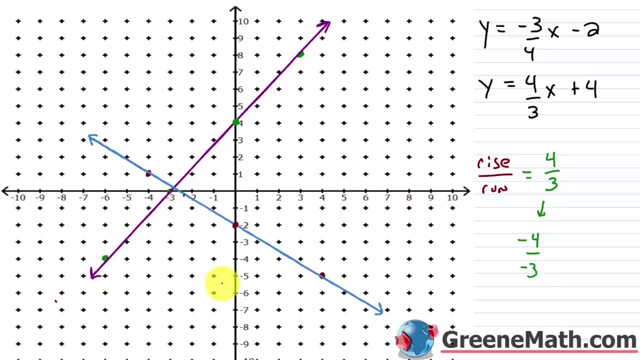 Okay. So let me graph this real quick: Okay, Okay, Okay, Okay, Okay, Okay. So one thing I want to draw your attention to: If you look at that point of intersection, you create a 90-degree angle there. Okay, This is a 90-degree angle And you can really 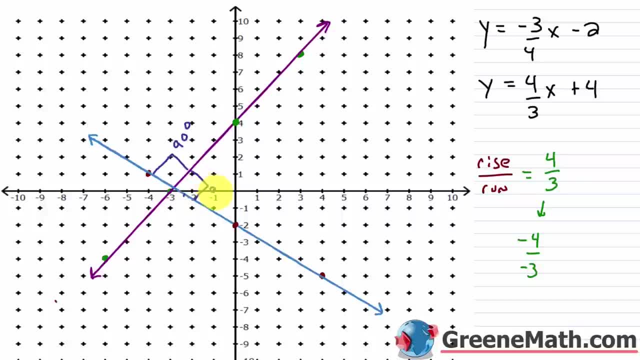 look at any of these and draw that. So this is also a 90-degree angle. This is also a 90-degree angle, And this is also a 90-degree angle. So it's all the way around. Let me make that a little better. 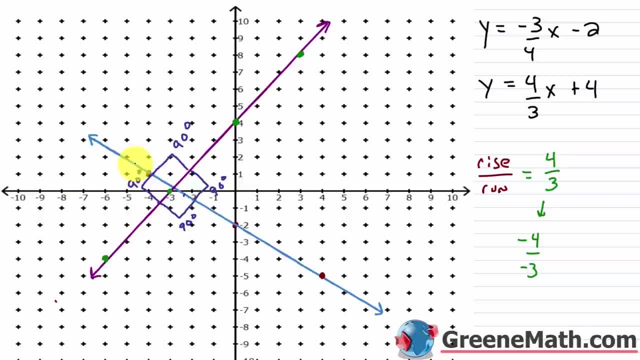 again, if you have two non vertical lines and you multiply the slopes together and you get negative one as a result, those two lines are perpendicular- you'll have a situation just like this one. All right, let's take a look at another one. We have x plus five y equals negative 10.. 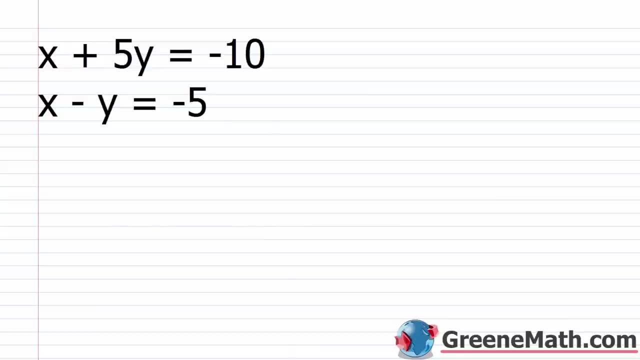 And we have: x minus y equals negative five. So again, I'm going to solve each one for y. So I'm gonna start out with this one. So we have x plus five, y equals negative 10.. I'm going to subtract x away from each side and I'll have five. y is equal to negative x. 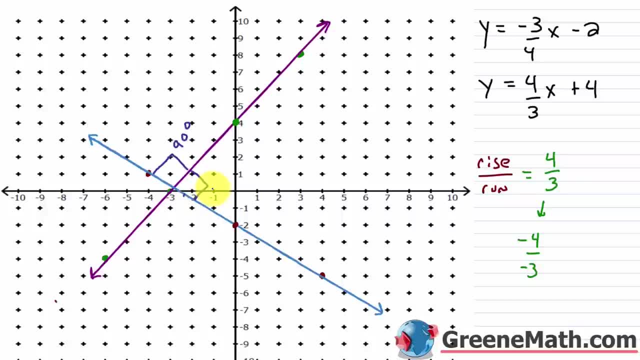 And you could really look at any of these and draw that. So this is also a 90-degree angle. This is also a 90-degree angle. And this is also a 90-degree angle. So it's all the way around. Let me make that a little better. OK. All right. 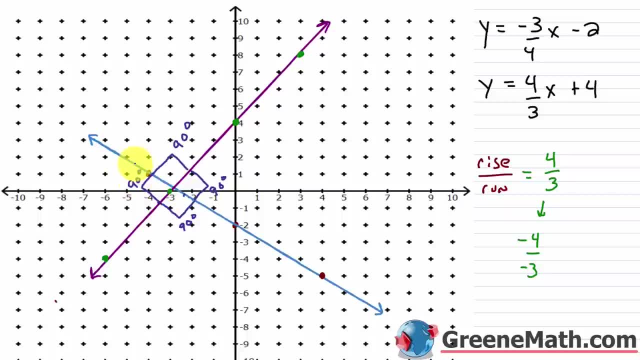 So again, if you have two non-vertical lines, and you multiply the slopes together, and you get negative 1 as a result, those two lines are perpendicular. 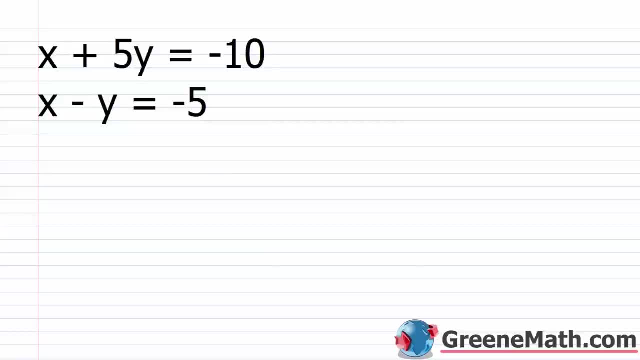 You'll have a situation just like this one. All right. 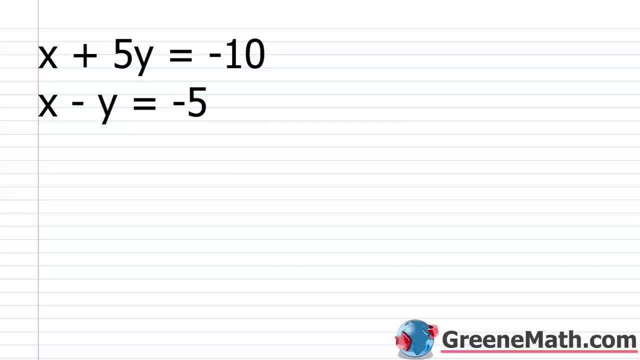 Let's take a look at another one. We have x plus 5y equals negative 10. And we have x minus y equals negative 5. So again, I'm going to solve each one for y. 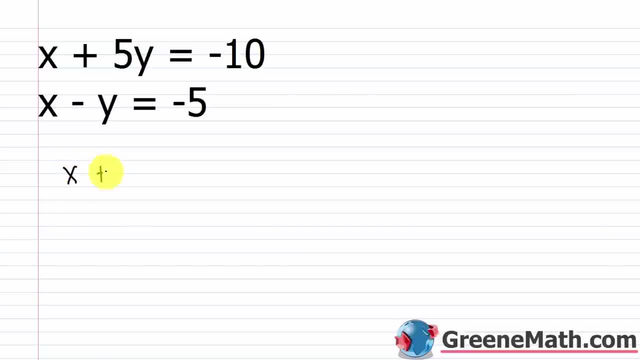 So I'm going to start out with this one. So we have x plus 5y equals negative 10. And we have x minus y equals negative 5. 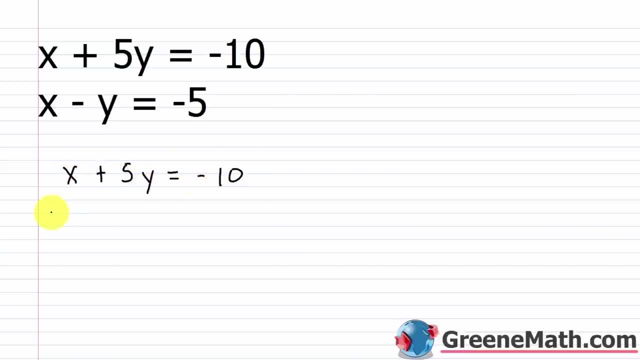 So again, I'm going to solve each one for y. So I'm going to start out with this one. So now I'm going to write negative 10. I'm going to subtract x away from each side. 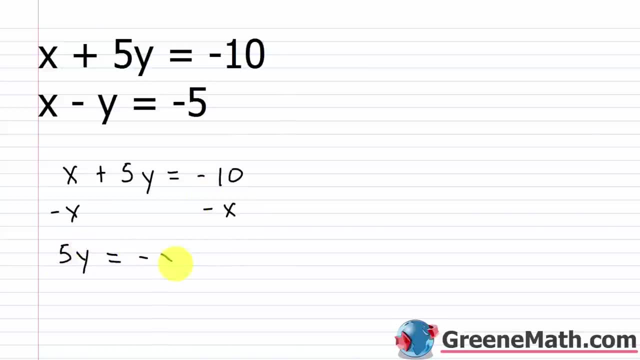 And I'll have 5y is equal to negative x minus 10. I will divide each side of the equation by 5. Let me scroll down a little bit. 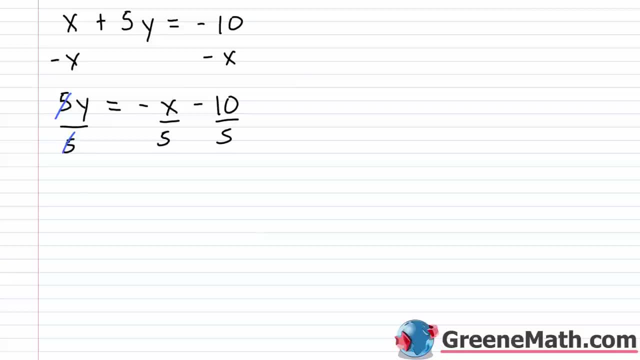 So this is going to cancel. And what are we going to have? We're going to have y is equal to. 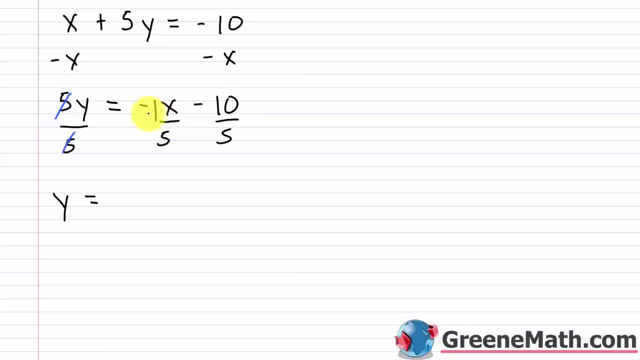 We have negative x over 5. Remember, I can write a 1 there. So it's the same as negative 1 fifth. Negative 1 fifth. 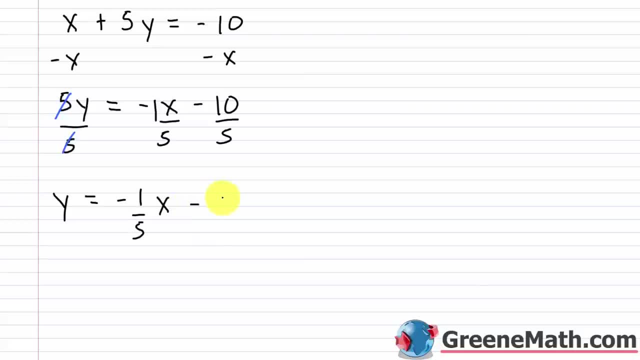 times x and then minus 10 over 5 we can think of as minus 2 right or plus negative 2 because 10 over 5 is 2. So then I have my equation in slope intercept form so I know the slope is negative one-fifth the y-intercept will occur at 0 comma negative 2. Let me erase all this 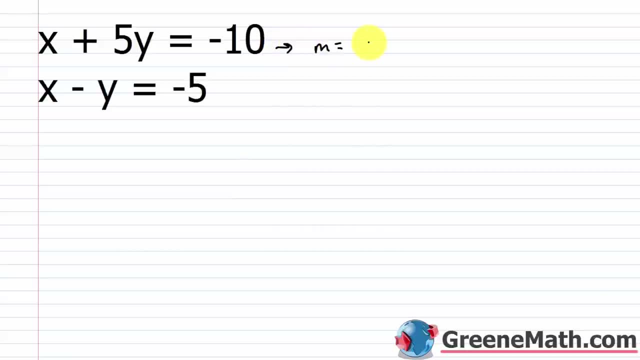 so then m is equal to negative one-fifth and again the y-intercept the y-intercept 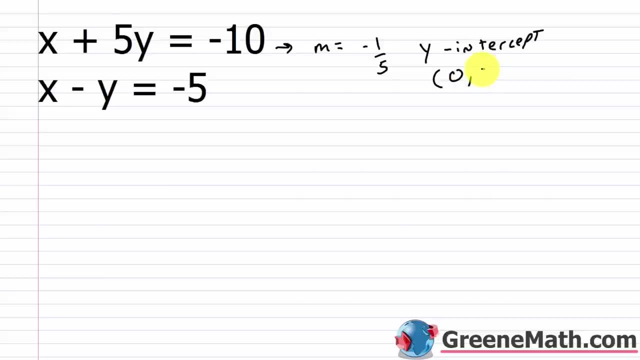 will occur at the point 0 comma negative 2. All right for this one pretty easy to solve for y we have x minus y equals negative 5. I just subtract x away from each side so that's gone I'll have negative y is equal to negative x minus 5. I just have a negative out in front of y that's keeping 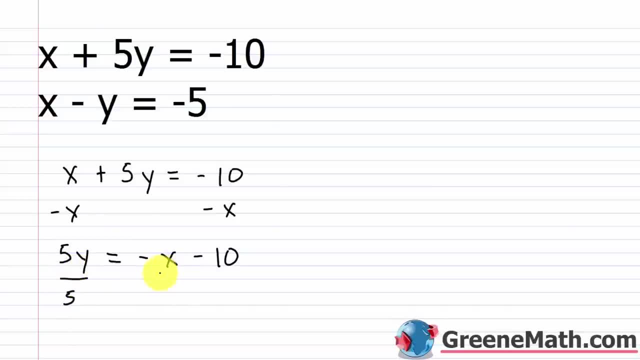 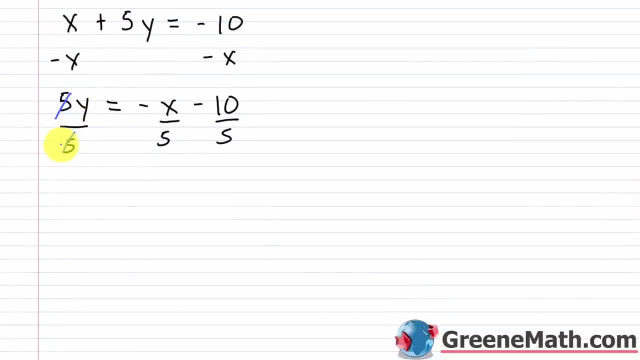 minus 10.. I will divide each side of the equation by five. Let me scroll down a little bit. So this is going to cancel, And what are we going to have? we're going to have: y is equal to. we have negative x over five, remember? I can write a one there, So it's the same as negative. 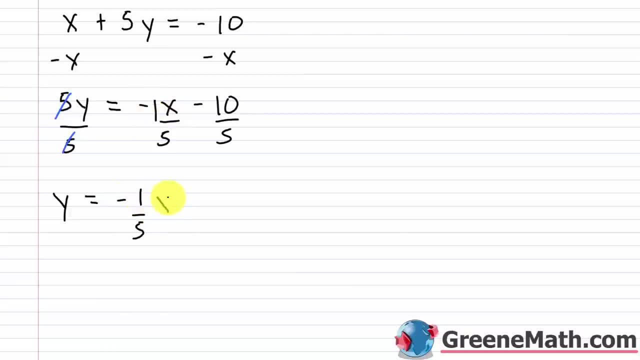 one fifth negative one fifth times negative x over five. So we have negative x over five times x and then minus 10 over five we can think of as minus two right, or plus negative two, because 10 over five is two. So then I have my equation in slope intercept form, So I know the 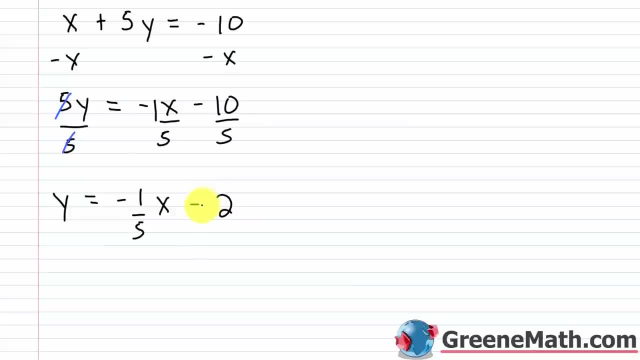 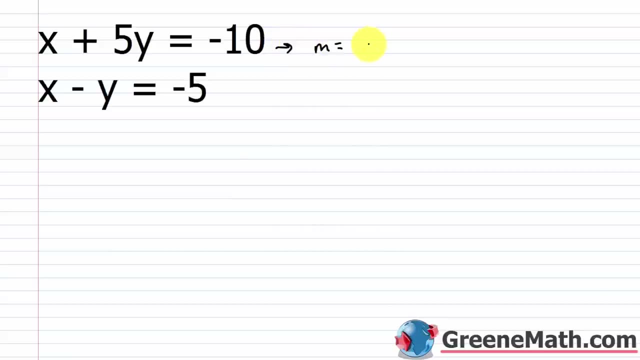 slope is negative one. fifth, the y intercept will occur at zero comma, negative two. Let me erase all this. So then m is equal to negative one. fifth, And again the y intercept. the y intercept will occur at the point zero comma negative two. All right for this one, pretty easy to solve for y: 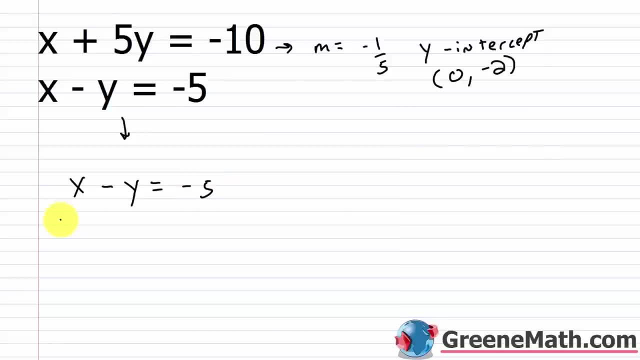 we have x minus y equals negative five. I just subtract x away from each side, So that's gone. I'll have negative. y is equal to negative x minus five. just have a negative out in front of y. that's keeping y from being by itself, So I can think of this as negative one times y. So in 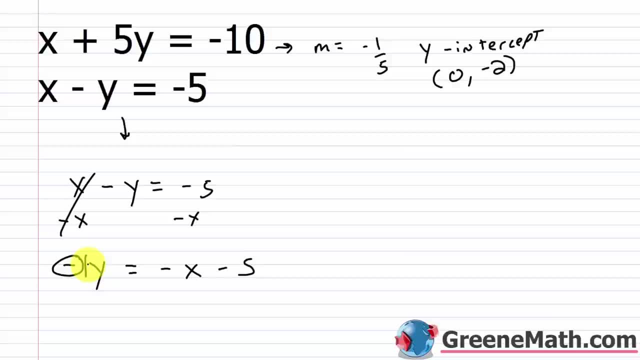 order to change the sign of that from negative to positive, I can divide it by negative one, fifth by negative one, or I can multiply by negative one, But I've got to do it to both sides of the equation. So let's multiply both sides of the equation by negative one, And so negative one. 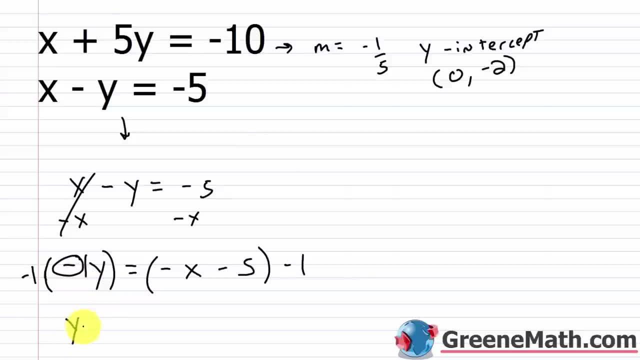 times negative. one is one, So I'd have one y or just y is equal to negative. one times negative. x is x, And then negative one times negative. five is plus five. So we get y equals x plus five. So my slope here is going to be one right, Because if I just have 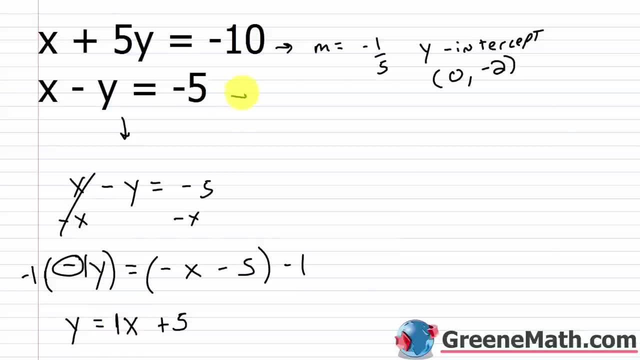 x by itself. it's got an invisible one next to it. So in this particular case m is equal to one And the y intercept occurs at zero comma five. So what can we say about these two lines here? Are they parallel? 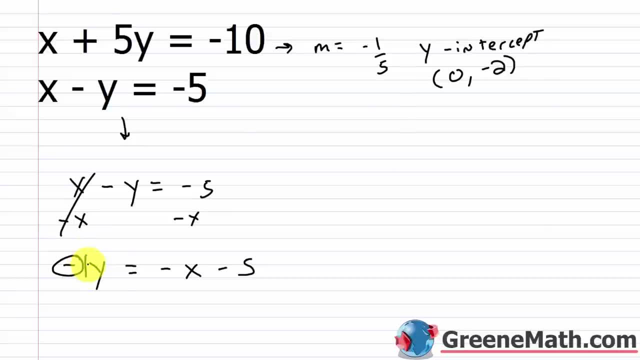 y from being by itself so I can think of this as negative 1 times y. So in order to change the sign of that from negative to positive I'm going to have to do a little bit of a workaround. So I'm going to have to divide by negative 1 or I can multiply by negative 1 but I've got to do it to both sides of the equation. So let's multiply both sides of the equation by negative 1 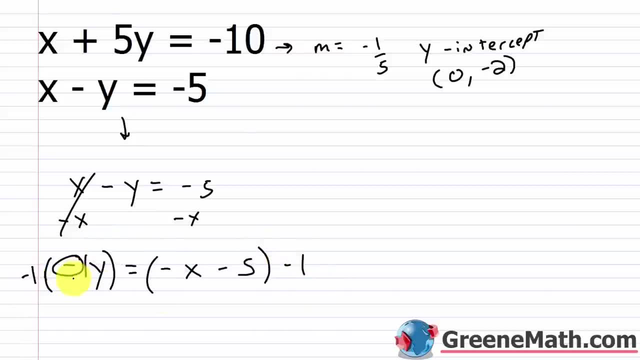 and so negative 1 times negative 1 is 1 so I'd have 1y or just y this is equal to negative 1 times negative x is x and then negative 1 times negative 5 is plus 5. So we get y equals x plus 5 so my slope here is going to be 1 right. 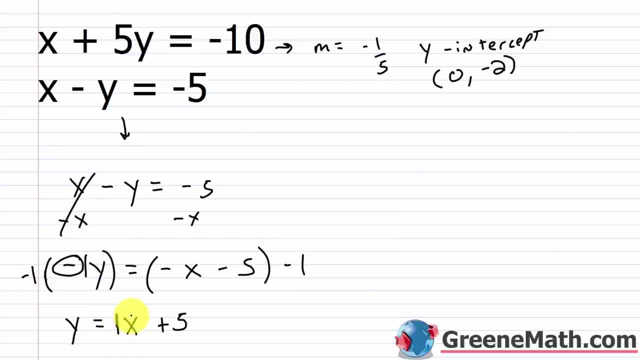 Because if I just have x by itself it's got an invisible 1 next to it. So in this particular case m is equal to 1 and the y-intercept occurs at 0 comma 5. So what can we say about these two lines 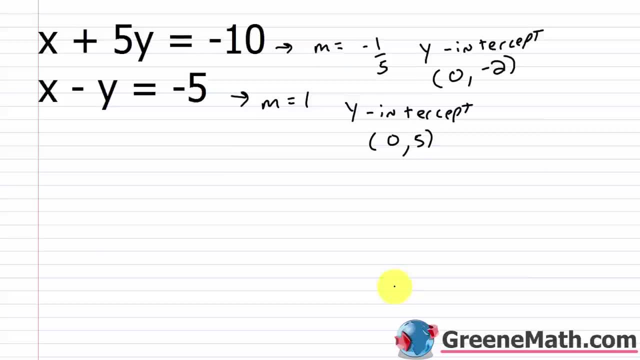 here? Are they parallel? Well the slopes are different. I have a slope here that's negative 1 fifth. I have a slope here that's 1. That's not the same so they're not parallel. Are they perpendicular? No you can tell that right away because if I multiply negative 1 times negative 1 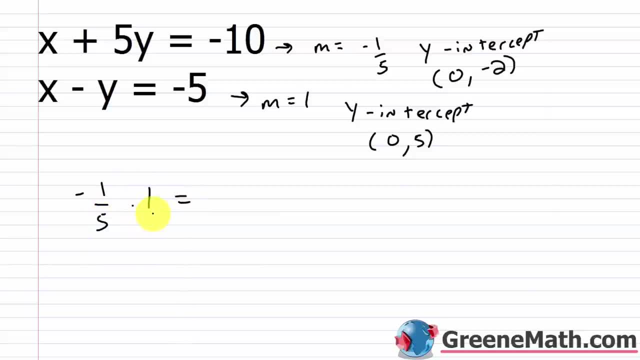 is 1. So I'm going to have x minus y equals negative 1 times negative 1. So I'm going to have x minus y equals negative 1 times negative 1. So negative 1 times negative 1 equals negative 1. So negative 1 fifth times 1 anything times 1 is just itself. So negative 5th times 1 is just negative 1 fifth. 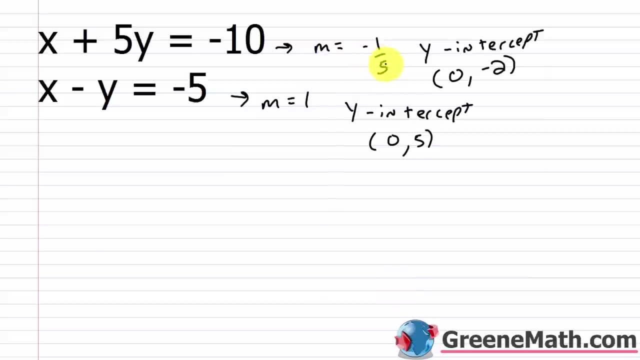 Well, the slopes are different. I have a slope here that's negative one. fifth, I have a slope here that's one that's not the same. So they're not parallel. Are they perpendicular? No, you can tell that right away, Because if I multiply, 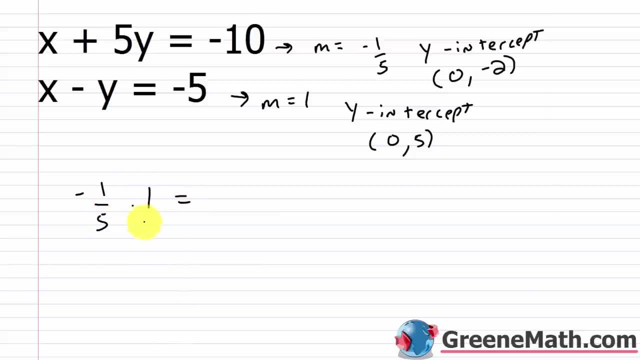 negative one fifth times one. anything times one is just itself. So negative fifth times one is just negative one fifth right. So these lines are also not going to be perpendicular, So in this case we would write neither right. We're going to say neither All right, so we want to write the. 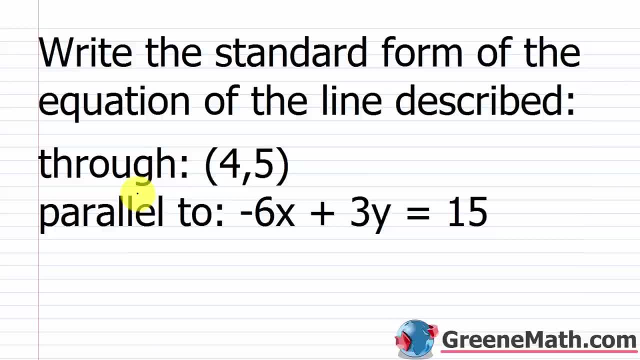 standard form of the equation of the line described. All right, so as you get further into this section on parallel and perpendicular lines, you're going to see a few problems like this, where you're given a point on the line and you're going to get a point on the line. 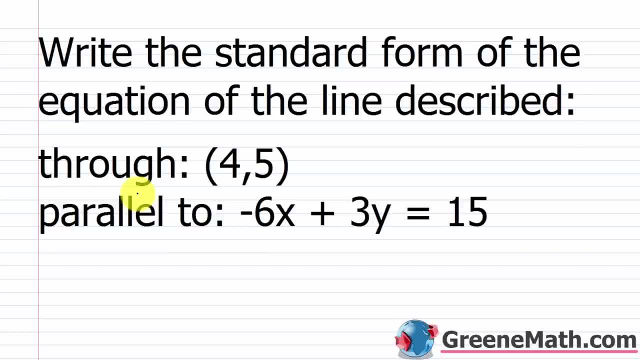 and you're given an equation that it's parallel to or perpendicular to, and you're expected to be able to write the equation of the line And they'll tell you which form they want it in. They'll say, okay, we want it in slope, intercept form, standard form, whatever they want, right? So in this case, 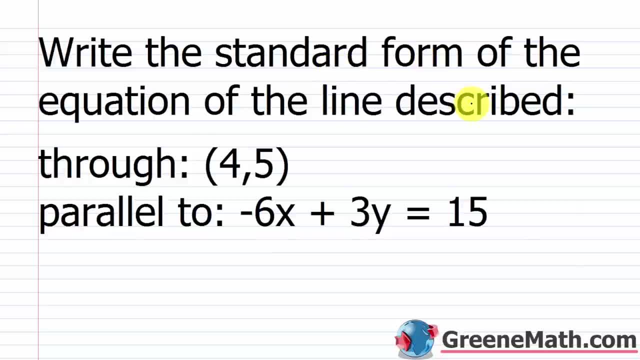 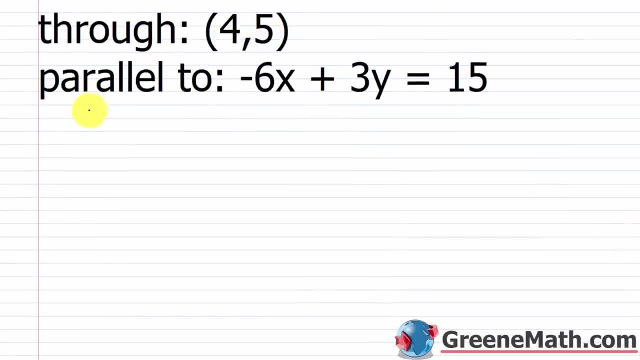 we want to write the standard form of the equation of the line described. So we're given this information here. It's through the point four, comma five, And it's parallel to this equation. here negative six plus three y equals 15.. So, remember, if I have a slope and I have a point on the line, I can use. 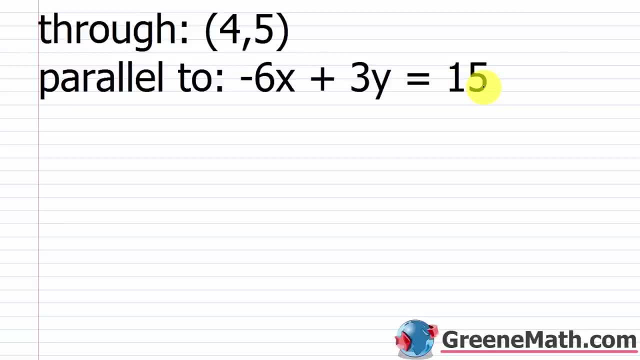 my point: slope form. okay, But before we get to that, we don't know what the slope is until we figure out a little information with this equation here. right, We don't know the slope, Slope equals what? So remember, if two lines are parallel, okay, they have the same slope. So you're meant. 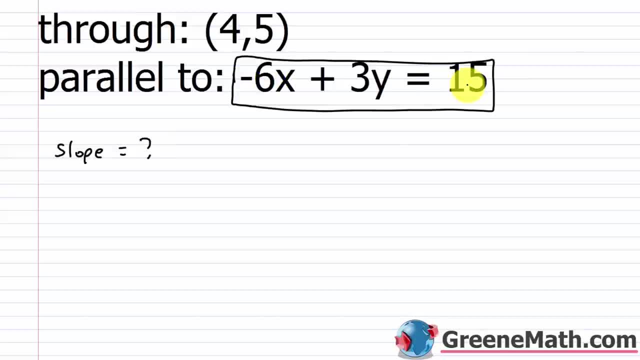 to look at this type of problem and say, okay, well, if I solve this for y, I can figure out the slope. And then I know my slope and I know my point, so I can use point slope form. So let's start out by just putting this in: slope intercept. 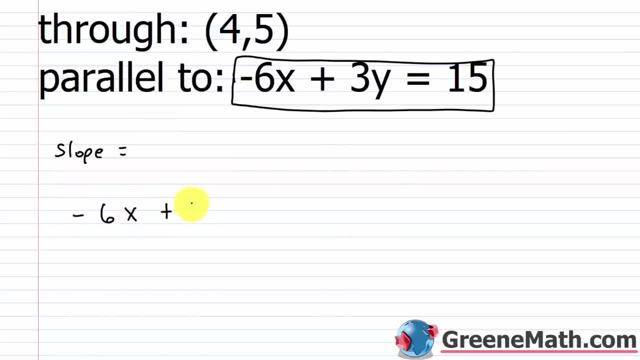 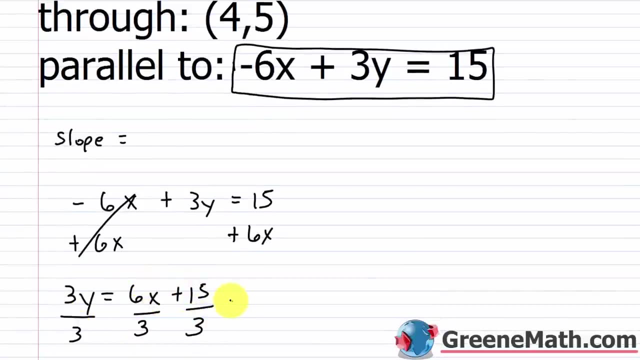 form So negative. six x plus three y equals 15.. Add six x to both sides of the equation, That's gone. Three y equals six x plus 15.. Divide this by three, divide this by three and this by three, So I get. 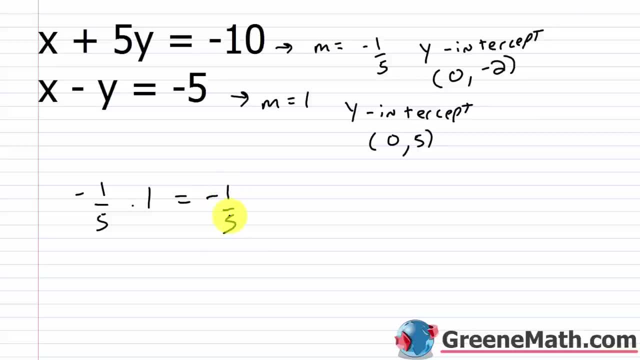 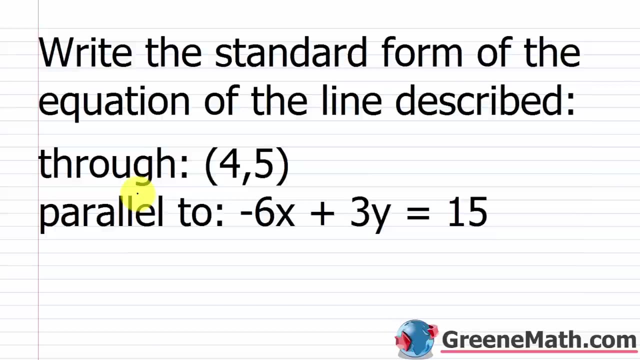 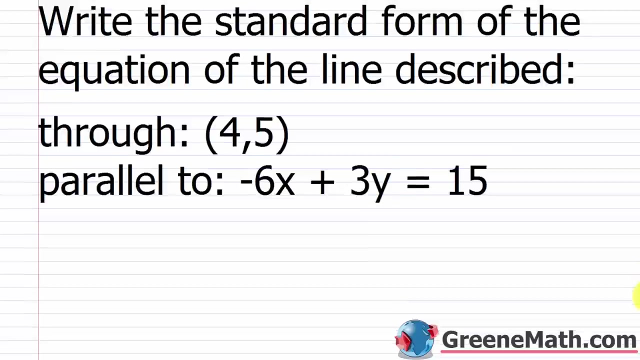 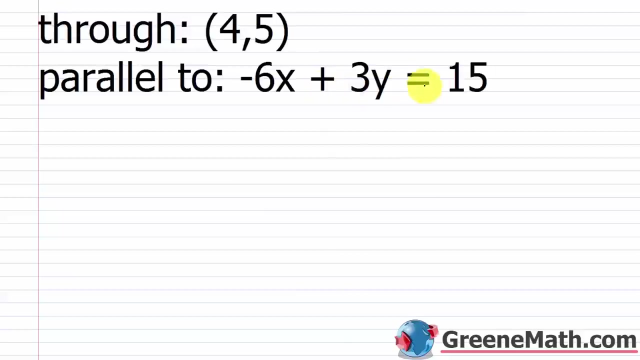 So these lines are also not going to be perpendicular. So in this case we would write neither. We're going to say neither. So we want to write the standard form of the equation of the line described. So as you get further into this section on parallel and perpendicular lines you're going to see a few problems like this. Where you're given a point on the line and you're given an equation that it's parallel to or perpendicular to and you're expected to be able to write the equation of the line and they'll tell you which form they want it in they'll say okay we want it in slope intercept form standard form whatever they want right so in this case we want to write the standard form of the equation of the line described so we're given this information here it's through the point four comma five and it's parallel to this equation here negative six x plus three y equals 15 so remember if i have a slope and i have a point on the line i can use my point slope form okay but before we get to that we don't know what the slope is until we figure out a little information with this equation here right we don't know the slope slope equals what so remember if two lines are parallel okay they have the same slope so 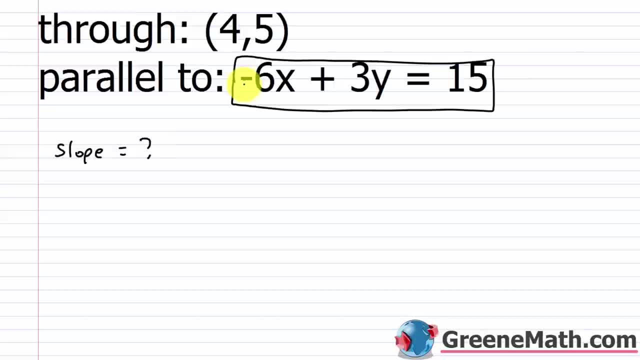 you're meant to look at this type of problem and say okay well if i solve this for y i can figure 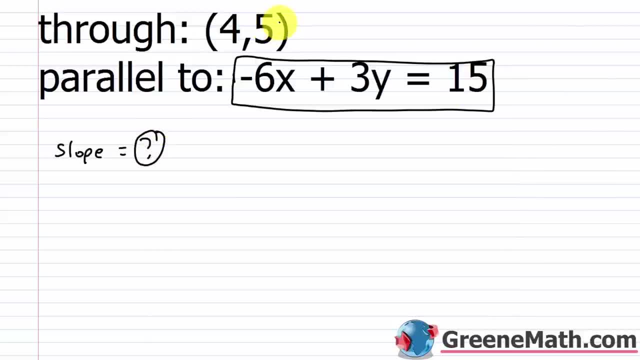 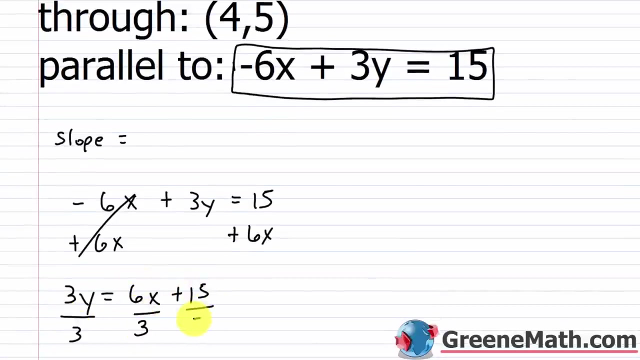 out the slope and then i know my slope and i know my point so i can use point slope form so let's start out by just putting this in slope intercept form so negative 6x plus 3y equals 15 add 6x to both sides of the equation that's gone 3y equals 6x plus 15 divide this by 3 divide this by 3 and this by 3 so i'll get y equals six over three is two so 2x plus 15 over three is five so y equals 2. 6. 2x 1. 1. 2. 3. 4. 6. 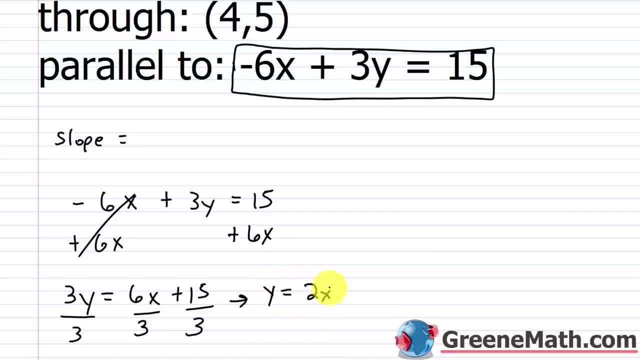 y equals six over three is two. so two x plus 15 over three is five. So y equals two x plus five. Remember, in slope intercept form y equals m, x plus b. M is your slope, So two. here is the slope. 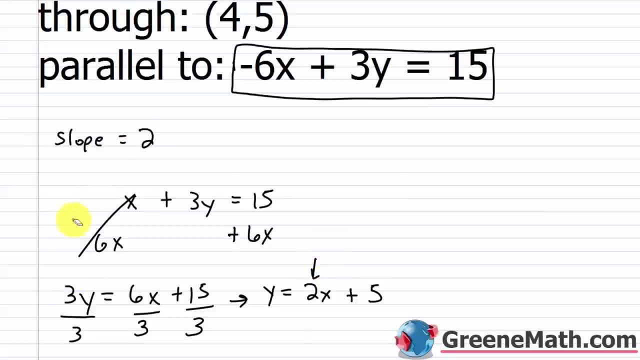 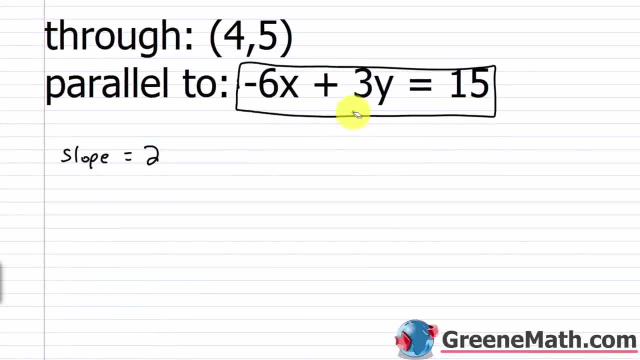 So the slope is two. Now, this is very important. It trips a lot of students up. If you're a little confused about this topic, you're not doing anything with this equation here. I can line it out once I know what the slope is. So I can line it out once I know what the slope is, So I can. 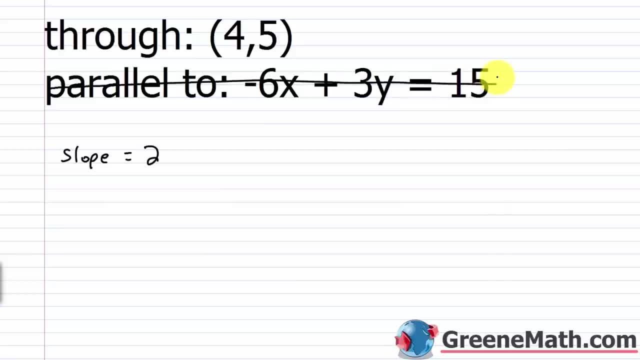 line it out. once I know what the slope is, I don't need it. It's irrelevant to me. Just get rid of it, because it's going to confuse you. You only need it to figure out what the slope is going to be in the equation that you're asked to write. I now know what the slope is because it was. 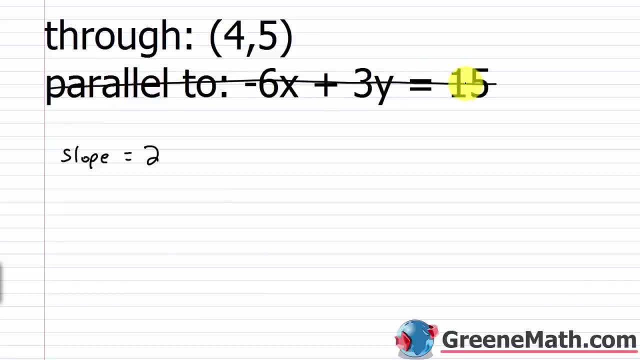 parallel to this equation. I took the equation, figured out what the slope was. I don't need it anymore. So I have my slope and I have my point. And again, when we have a slope and a point on the line, we use point slope form. 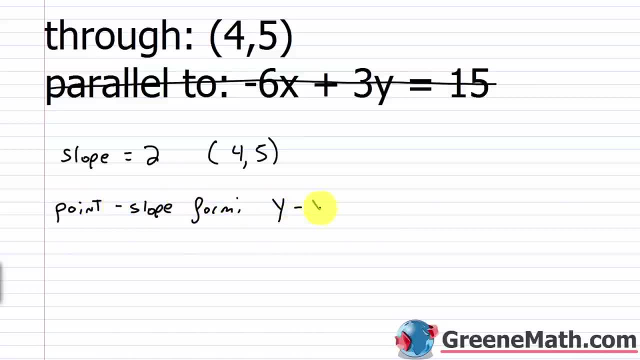 Which is what It's. y minus y sub 1 is equal to m. the slope times the quantity x minus x sub 1.. Where this y sub 1 and the x sub 1 are the given values from that point. So this is x sub 1.. This 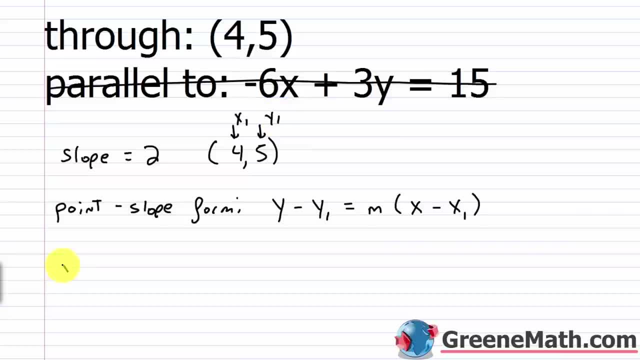 is y sub 1.. And now we just plug in, We'd have y minus y sub 1,, which is 5, is equal to m, which is 2.. That's your slope times the quantity x minus x sub 1.. 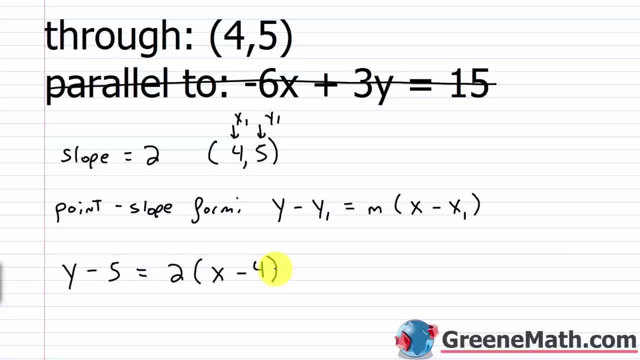 One is 4.. Now, if they're asking for point slope form, you're done, But they didn't. They actually asked for standard form. So what we're going to do is we're going to solve this for y first. So I'm going to have: y minus 5 equals 2 times x is 2x, And then 2 times negative 4 is negative 8.. 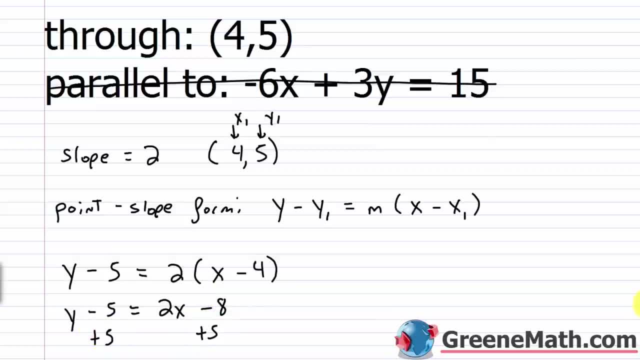 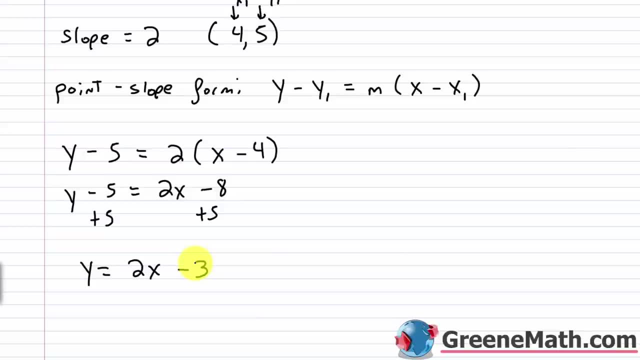 Add 5 to both sides of the equation, I'll get y equals 2x minus 3.. Now the problem with this is: This still isn't standard form. Again, this is slope-intercept form. If it's solved for y, this is slope-intercept form. 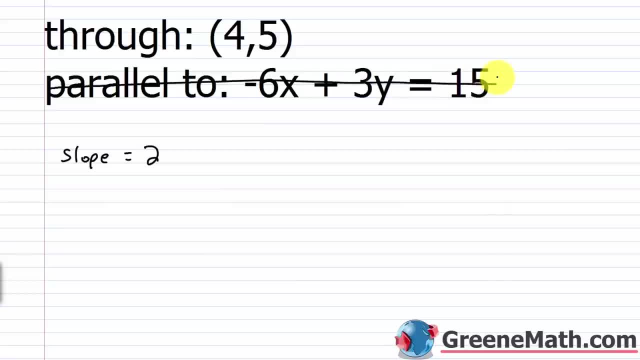 equation here. I can line it out once I know what the slope is. I don't need it. It's irrelevant to me. Just get rid of it because it's going to confuse you. You only need it to figure out what the slope is going to be in the equation that you're asked to write. I now know what the slope is because it was parallel to this equation. I took the equation, figured out what the slope was. I don't need it anymore. So I have my slope and I have my point. And again, when we have a slope and a point on the line, we use point-slope form. Which is what? It's y minus y sub 1 is equal to m the slope times the quantity x minus x sub 1. Where this y sub 1 and the x sub 1 are the given values from that point. So this is x sub 1. This is y sub 1. And now we just plug in. We'd have y minus y sub 1, which is 5, is equal to m. 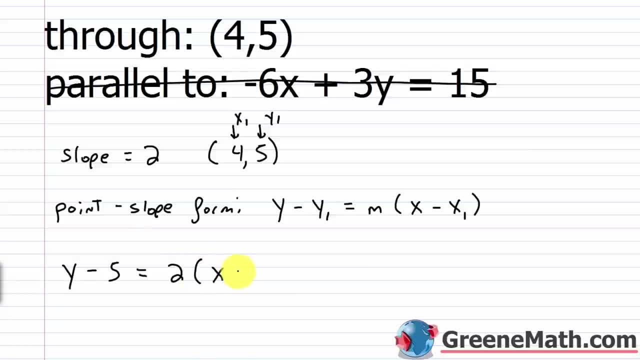 Which is 2. That's your slope times the quantity x minus x sub 1. x sub 1 is 4. Now, if they're asking for point-slope form, you're done. But they didn't. They actually asked for standard form. So what we're going to do is we're going to solve this for y first. So I'm going to have y minus 5 equals 2 times x is 2x. And then 2 times negative 4 is negative 8. Add 5 to both sides of the equation. 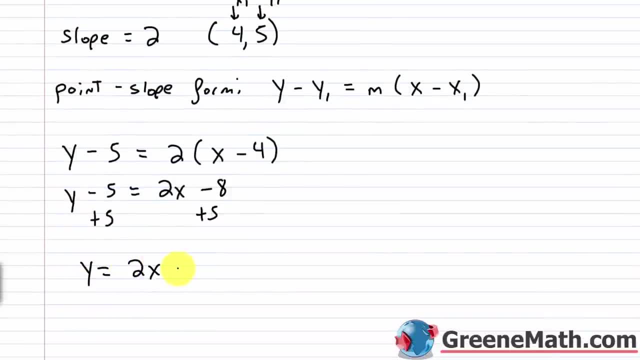 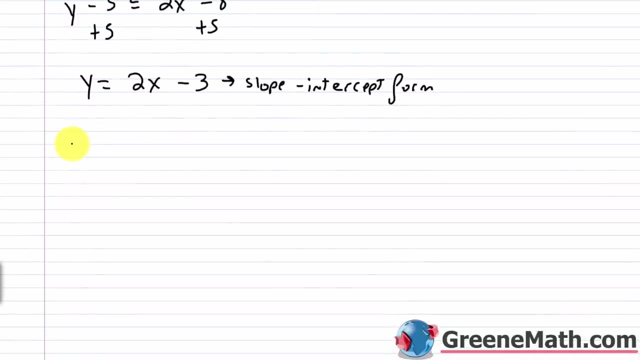 I'll get y equals 2x minus 3. Now, this still isn't standard form. Again, this is slope-intercept form. If it's solved for y, this is slope-intercept form. Very important you understand the difference between those. Now, for standard form, again, you want it to look like this. ax plus by equals c. And I know everybody has a different definition. 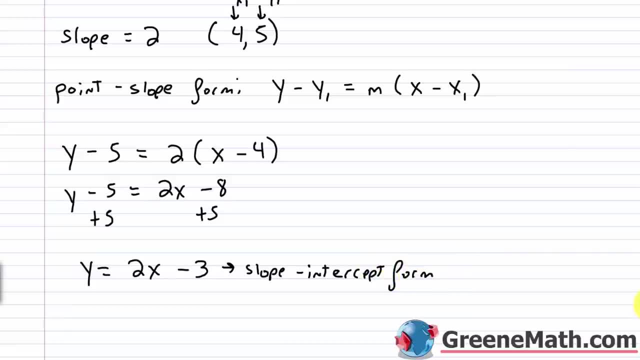 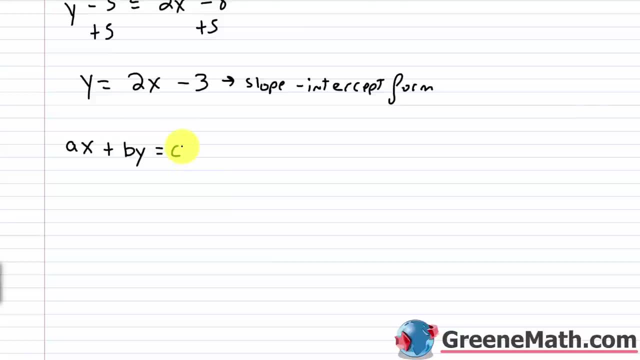 Very important. you understand the difference between those. Now for standard form again. you want it to look like this: Ax plus By equals C, And I know everybody has a different definition for that, but typically in high school you see it written like this: 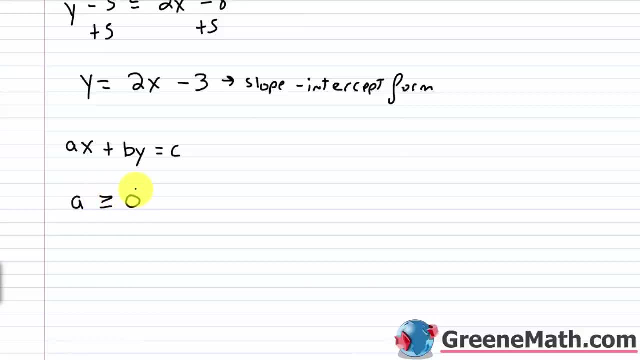 and you'll say that A has to be greater than or equal to 0. So it's either 0 or some positive value, And then A, B and C need to be integers, and A and B can't both be 0 at the same time. 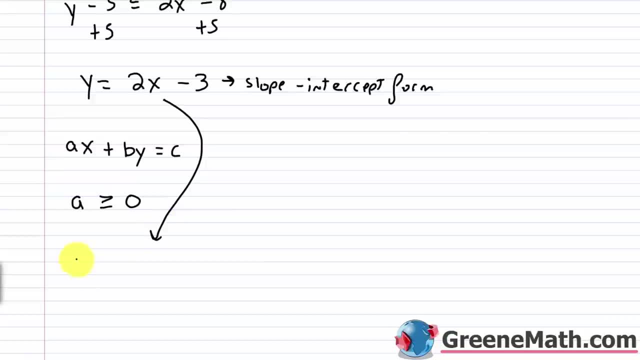 So, in order to make that happen, if I look at this, y equals 2x minus 3, I know I want to move this over here, So I would subtract it away from both sides, So I'd have negative 2x plus y equals negative 3.. 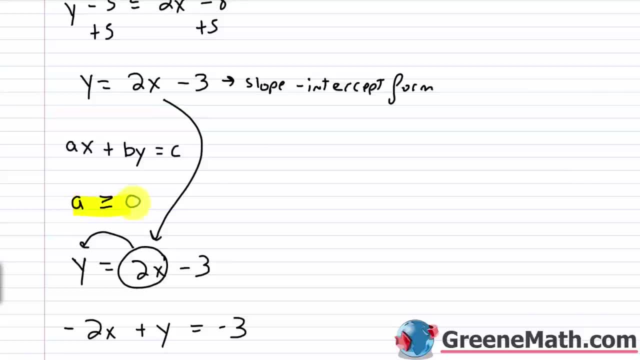 But according to my definition that I'm using, A has to be greater than or equal to 0. So to kind of clean this up, I just don't want that to be negative, So I can just multiply both sides of the equation by negative 1.. 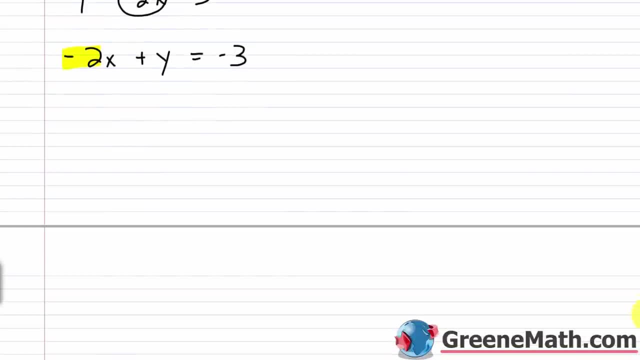 Very, very simple fix for that. So if I multiply this side by negative 1 and this side by negative 1, I'll end up with negative 1 times negative 2.. That's 2x and then negative 1 times y would be minus y. 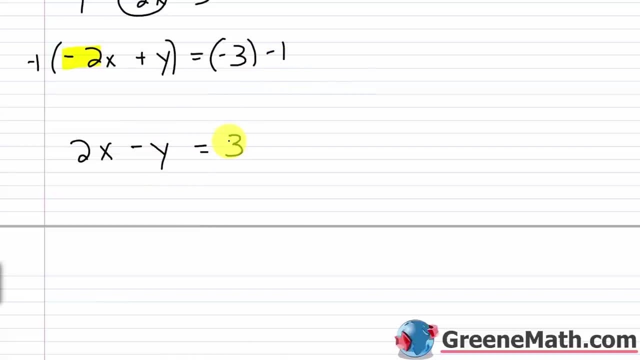 And this equals negative 3 times negative 1, which is 3.. So I get 2x. So I get 2x minus y equals 3.. So that would be the equation of the line in standard form that passes through the point 4, 5. 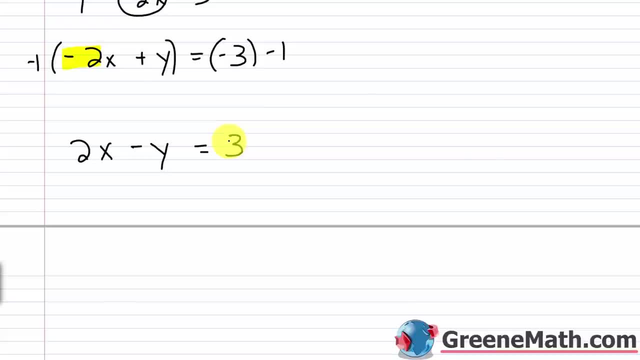 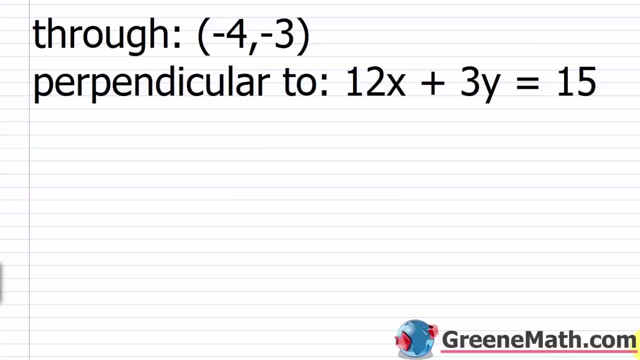 and is parallel to negative. 6x plus 3y equals 15.. All right, we're going to take a look at one more. So this one passes through the point: negative 4,, negative 3, and it's now perpendicular to 12x plus 3y equals 15.. 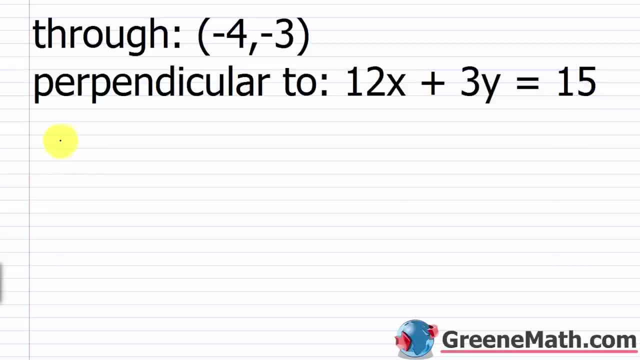 So again, I'm going to solve this for y. So let me start out by just saying we have 12x plus 3y. That equals 15.. I want to subtract 12x away from each side. That's going to go. 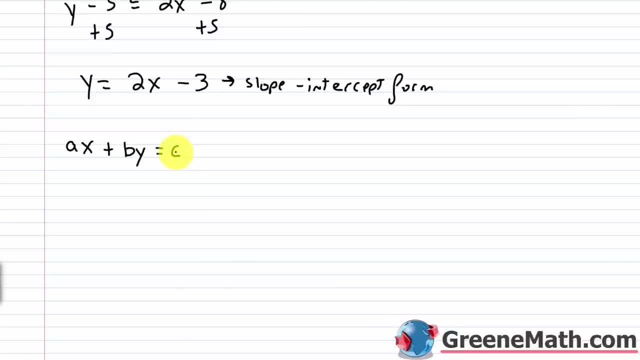 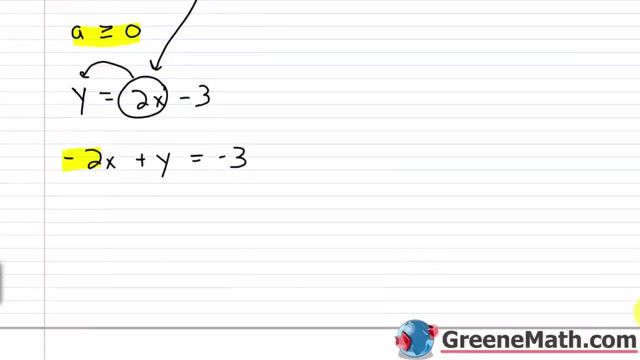 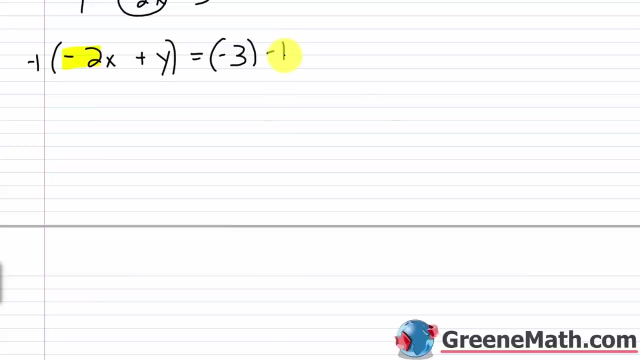 But typically, in high school, you see it written like this. And you'll say that a has to be greater than or equal to 0. So it's either 0 or some positive value. And then a, b, and c need to be integers. And a and b can't both be 0 at the same time. So in order to make that happen, if I look at this, y equals 2x minus 3, I know I want to move this over here. So I would subtract it away from both sides. So I'd have negative 2x plus y equals negative 2x minus 3. And then I'd have negative 3. But according to my definition that I'm using, a has to be greater than or equal to 0. So to kind of clean this up, I just don't want that to be negative. So I can just multiply both sides of the equation by negative 1. Very, very simple fix for that. So if I multiply this side by negative 1 and this side by negative 1, I'll end up with negative 1 times negative 2. 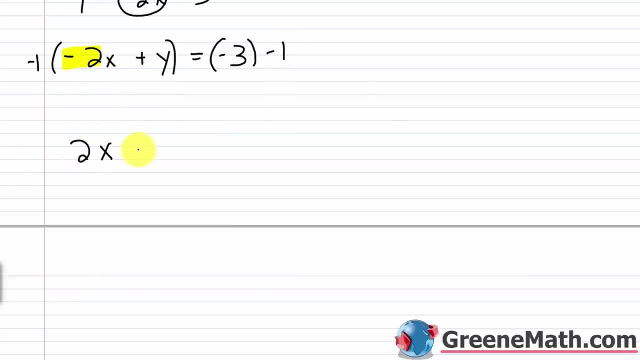 That's 2x. And then negative 1 times y would be minus y. This equals negative 3 times negative 1, which is 3. So I get 2x minus y equals 3. So that would be 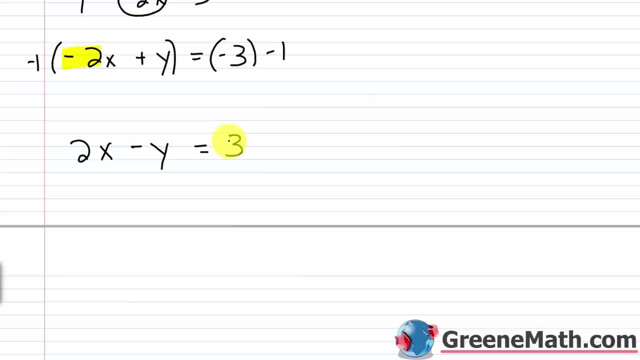 the equation of the line in standard form that passes through the point 4 comma 5 and is parallel 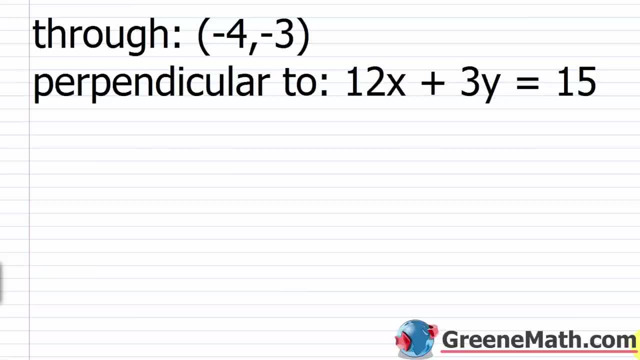 to negative 6x plus 3y equals 15. All right, we're going to take a look at one more. 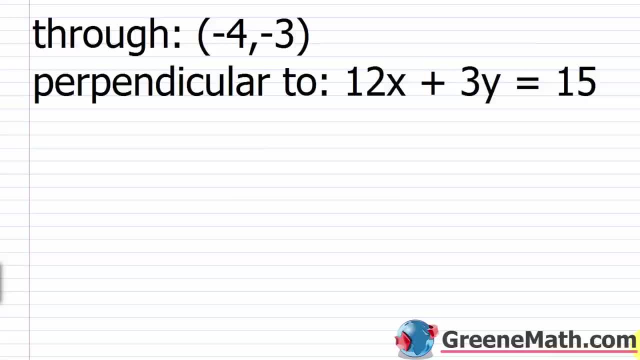 So this one passes through the point negative 4 comma negative 3. And it's now perpendicular to 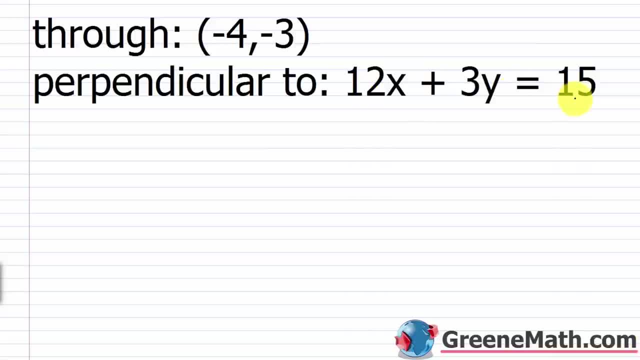 12x plus 3y equals 15. So again, I'm going to solve this for y. So let me start off with a problem. So I'm going to start off by just saying, OK, we have 12x plus 3y equals 15. I want to 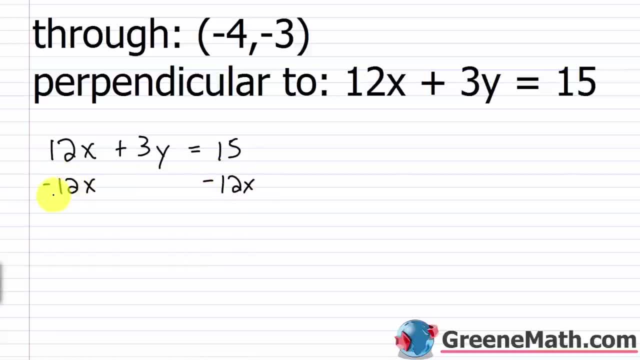 subtract 12x away from each side. That's going to go. And I'll have 3y is equal to negative 12x plus 15. And we're going to divide each side of the equation by 3. 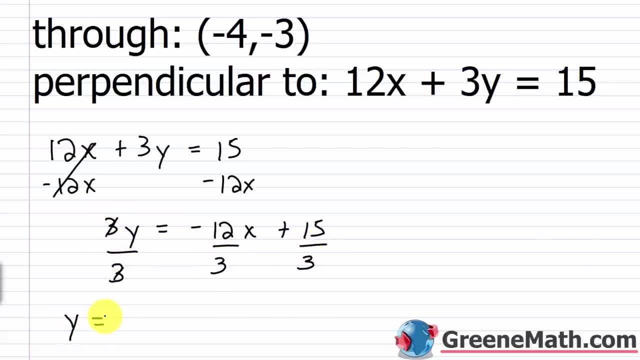 And what are we going to have? This will cancel. I'll have y is equal to negative 12 over 3 is negative 4, then times x. And then plus 3y is equal to negative 12x. And then plus 3y is equal to plus 15 over 3. That's plus 5. All right, so I'd have y equals negative 4x plus 5. Now, 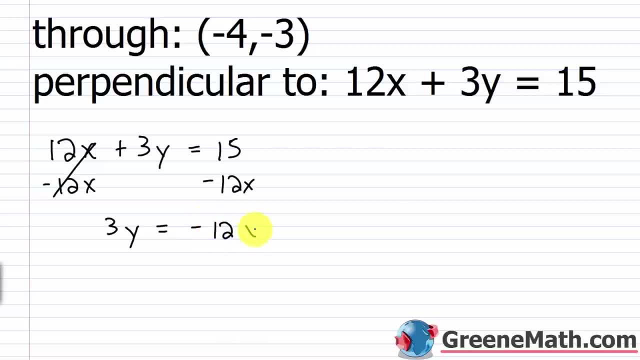 And I'll have: 3y is equal to negative 12x plus 15.. And we're going to divide each side of the equation by 3.. And what are we going to have? This will cancel. I'll have: y is equal to negative. 12 over 3 is negative 4,. 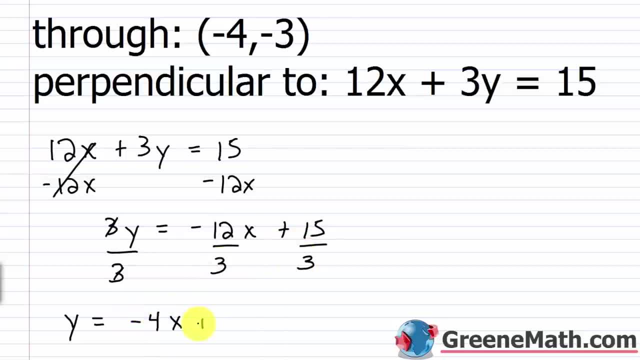 then times x, And then plus 15 over 3,, that's plus 5.. All right, so I'd have y equals negative 4x plus 5.. Now in the last example where we had parallel lines, it was easy because the slopes would just be the same. 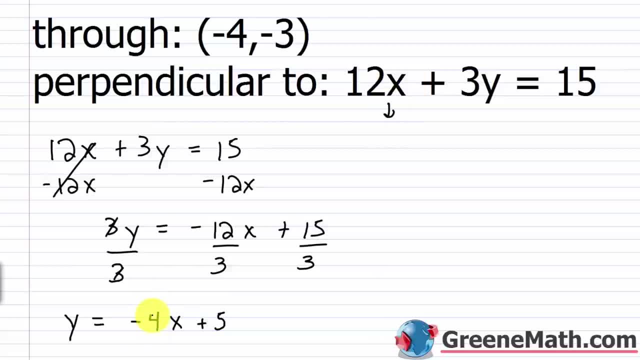 The slope for this line, as we can see, because it's in slope, intercept form m is equal to negative 4.. Now, with perpendicular lines it's a little bit more complex, but really it's still kind of easy. Perpendicular lines have a property. 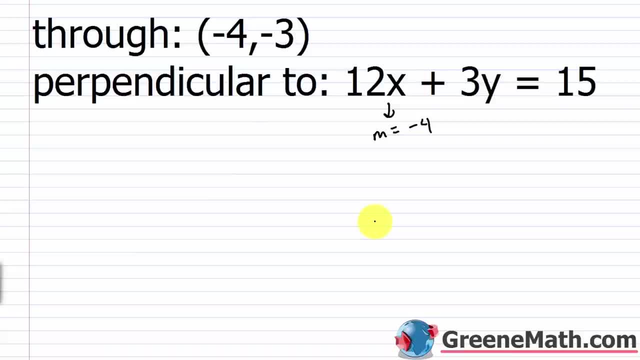 that says that the product of their slopes will be negative 1.. So that means negative 4 times some unknown slope- unknown slope right for the line we're trying to get to- is going to be equal to negative 1.. 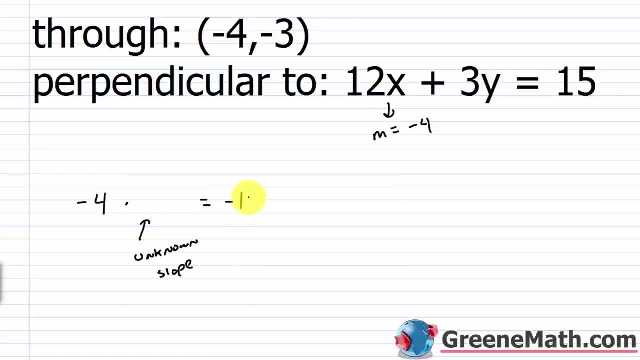 So I can use a variable here, right? I can always use a variable when I have something unknown, So let's use z. Now what I would do is if I had negative 4 times z equals negative 1, I would divide both sides of the equation, right? 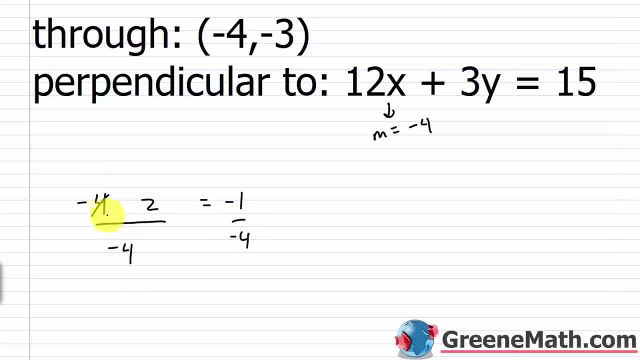 you kind of think about it this way- by negative 4.. This would cancel and z would equal negative 1 over negative 4, which is 1 fourth. So the slope I'm looking for is 1- fourth, Because if I take 1 fourth, 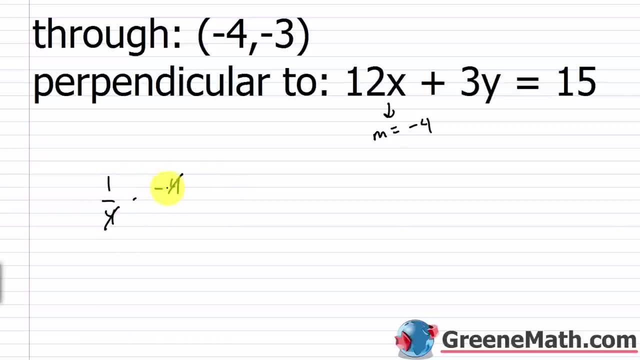 and I multiply it by negative 4, this would cancel. with this, I'd have 1 times negative 1, which would be negative 1.. That's exactly the property that we know from perpendicular lines. So now I know the slope of the line. 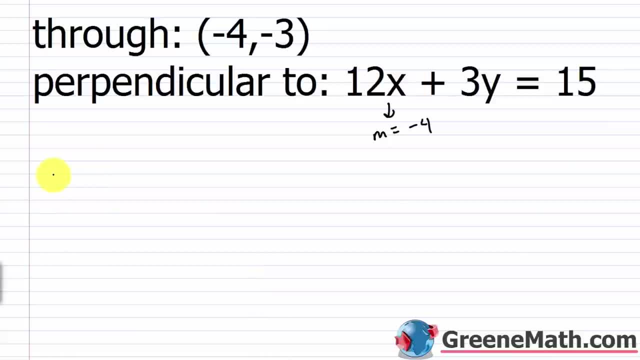 that I'm trying to put in standard form. Again, it's 1- fourth. So my m is equal to negative 1, which would be negative 1.. So my m is 1- fourth and my point on the line is negative 4 comma, negative 3.. 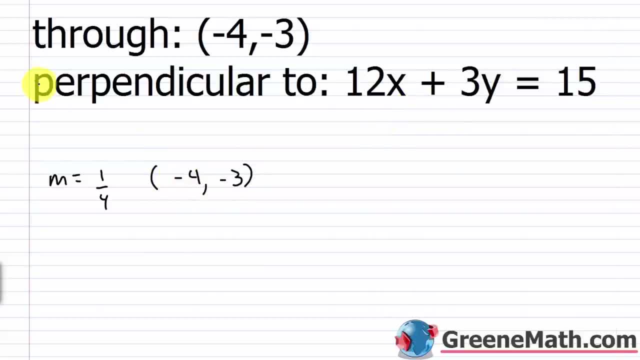 Now we are done with this equation here. We don't need it anymore. Line it out, Forget it exists. okay, You've gotten the information you need from it and just again forget about it. Now I'm gonna use my point slope form. 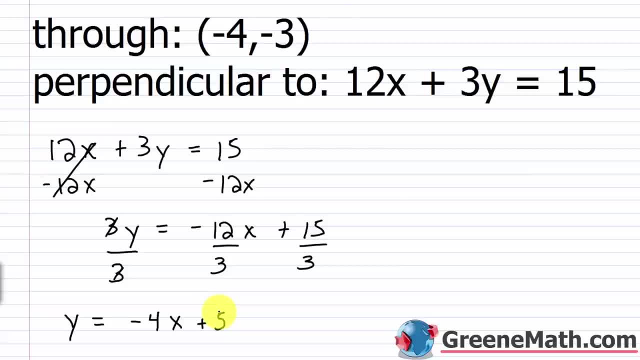 in the last example where we had parallel lines, it was easy because the slopes would just be the same. The slope for this line, as we can see, because it's in slope intercept form, m is equal to negative 4. Now, with perpendicular lines, it's a little bit more complex, but really, it's still kind of easy. Perpendicular lines have a property, that says that the product of their slopes will be negative 1. So that means negative 4 times some unknown slope, unknown slope, right, for the line we're trying to get to, 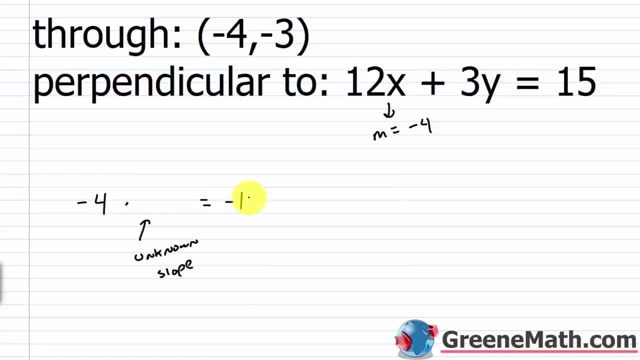 is going to be equal to negative 1. So I can use a variable here, right? I can always use a variable when I have something unknown. So let's use z. Now, what I would do is, if I had negative 4 times z equals negative 1, I would divide both sides of the equation, right? You kind of think about it this way, as by negative 4. This would cancel, and z would equal negative 1 over negative 4, which is 1 fourth. So the slope I'm looking for is 1 fourth, because if I take 1 fourth and I multiply it by negative 4, this would cancel 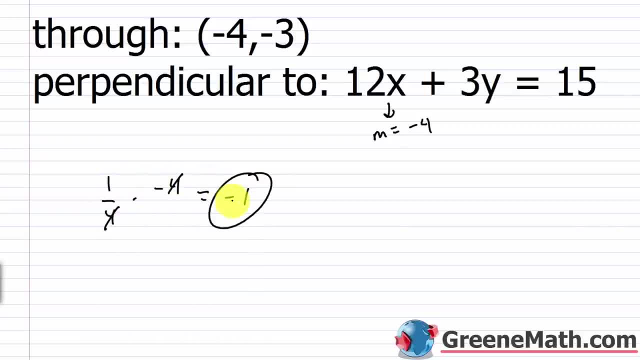 with this. I'd have 1 times negative 1, which would be negative 1. That's exactly the property that we know from perpendicular lines. So now I know the slope of the line that I'm trying to put in standard. 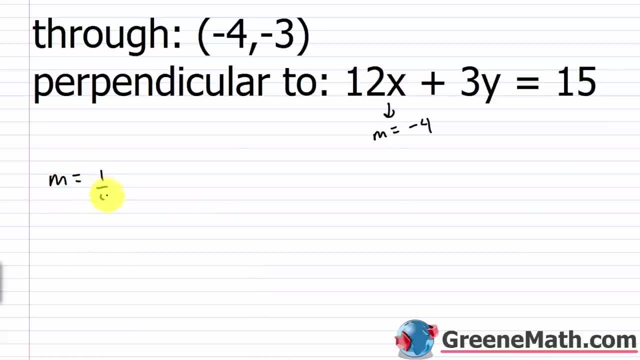 Again, it's 1 fourth. So my m is 1 fourth, and my point on the line is negative 4 comma negative 3. Now, we are done with this equation here. We don't need it anymore. Line it out. Forget it 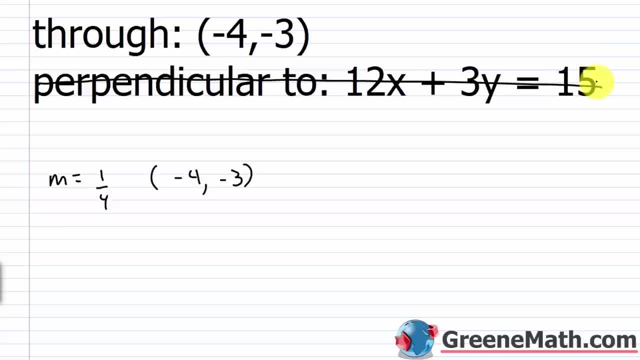 exists, okay? You've gotten the information you need from it, and just, again, forget about it. 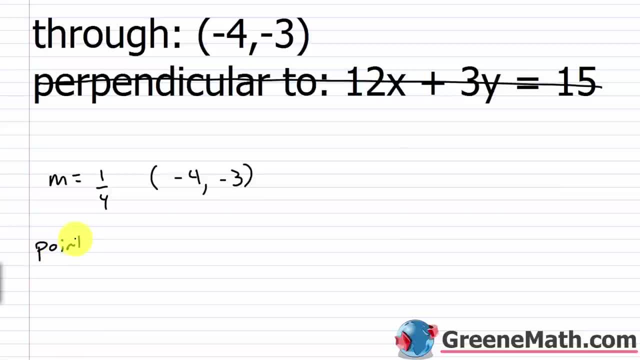 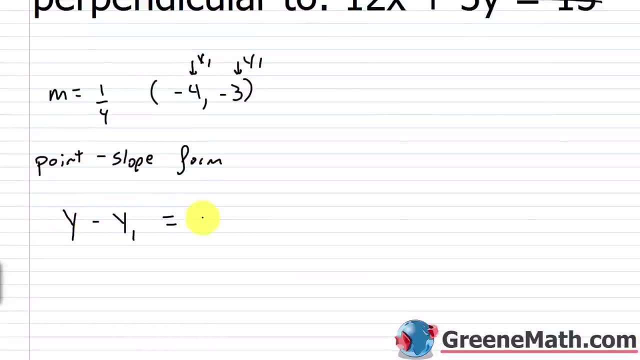 Now, I'm going to use my point-slope form. Point-slope form. Again, this is my x sub 1. This is my y. This is my y sub 1. And for point-slope form, again, it's y minus y sub 1 equals m times the quantity x minus x sub 1. I'm going to plug in a negative 3 right here. I'm going to plug in a negative 4 right here. So I'll have y minus a negative 3, so that's y plus 3, is equal to, and I forgot to say that I'm going to plug in a 1 fourth for m, so is equal to 1, 4 times this quantity x minus, and we're subtracting away negative 4, so I'm going to put plus 4. All right. So I'm going to solve this for y right now. Again, this is point-slope form. If it asked for that, we'd stop there. Solving it for y is pretty easy. We just have y plus 3 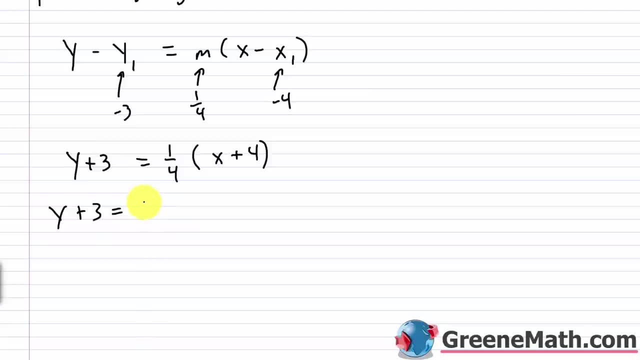 is equal to 1 fourth times x is just 1 fourth x, so you can put x over 4, and then plus 1 fourth times 4 is 1. So then I'd subtract 3 away from each side. 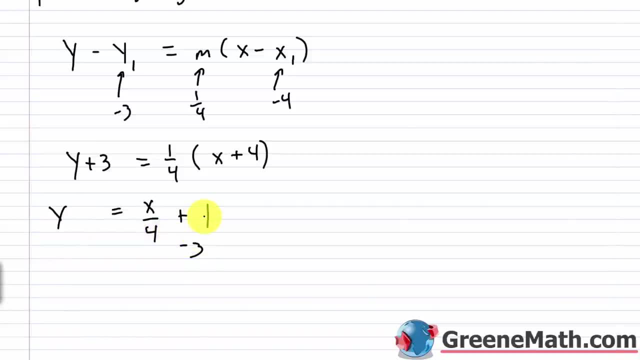 I'll go ahead and just do this. Like this, y equals x over 4 plus, and basically it's going to be negative 2, right? You can put 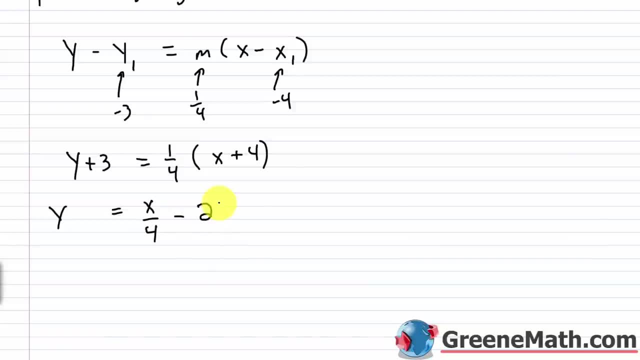 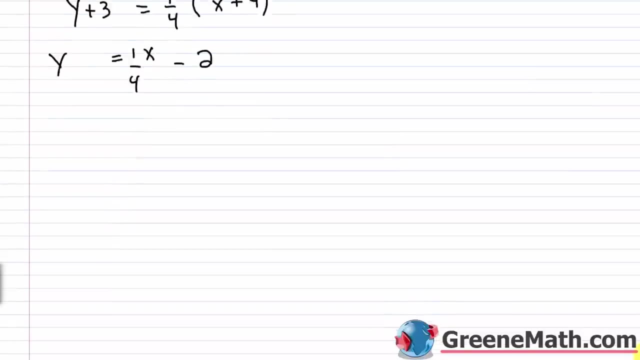 minus 2. So now I have the equation in slope-intercept form. y equals, and you could write it as x over 4, or you could write 1 fourth times x minus 2. It doesn't matter, and I want to put it in standard form, and again, let me kind of cover that definition again. Standard form looks like this, ax plus by equals c. 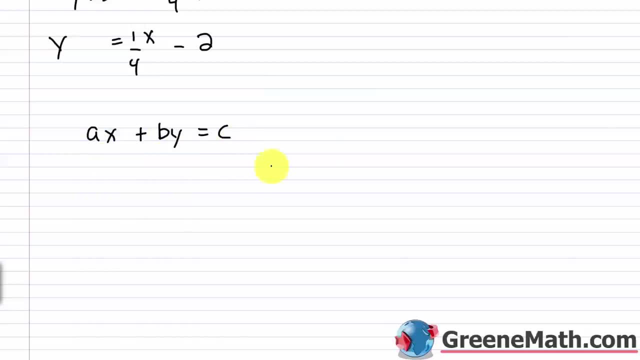 Again, where a, b, and c are integers, a and b are not both 0, and a is greater than or equal to 0. 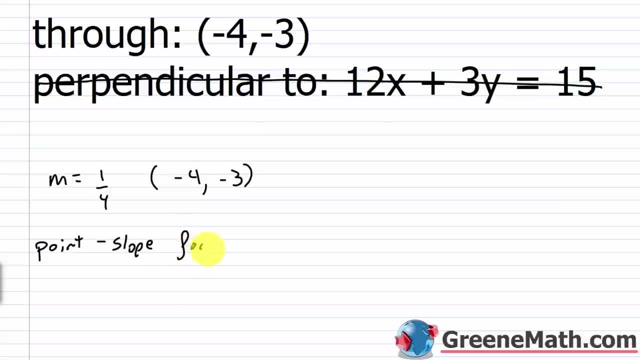 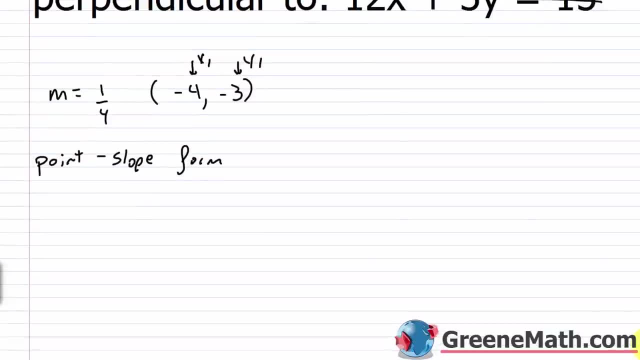 Point slope form: Again, this is my x sub 1.. This is my y sub 1.. And for point slope form, again, it's y minus y sub 1 equals m times the quantity x minus x sub 1.. I'm gonna plug in. 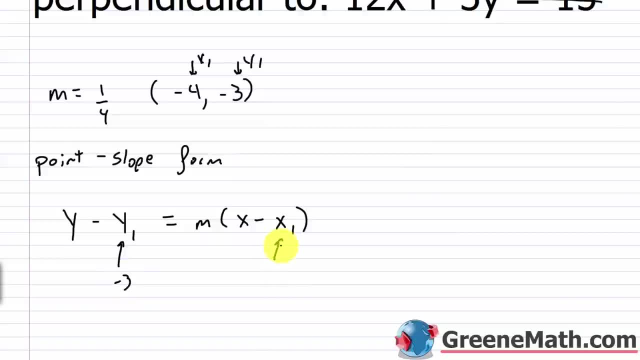 I'm gonna plug in a negative 3 right here. I'm gonna plug in a negative 4 right here. So I'll have y minus a negative 3, so that's y plus 3, is equal to- and I forgot to say that I'm gonna plug in a 1 fourth for m. 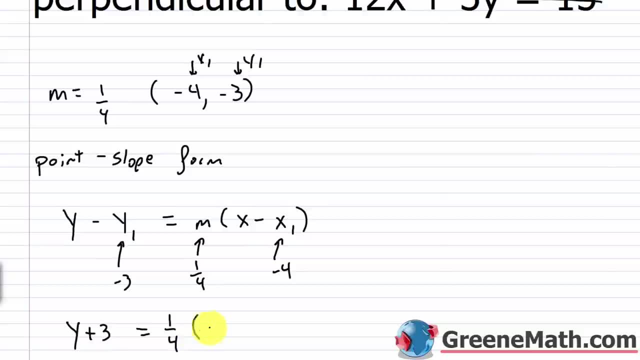 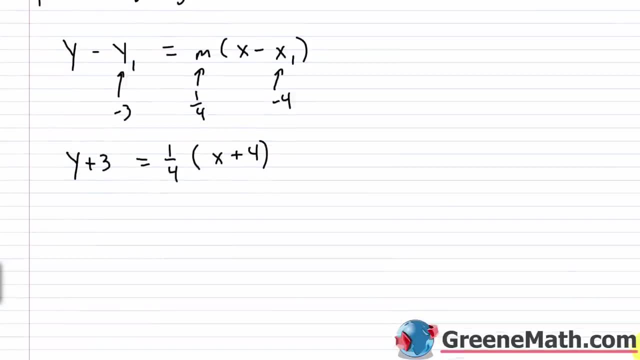 So is equal to 1, fourth times this quantity x minus, and we're subtracting away negative 4, so I'm gonna put plus 4.. All right, So I'm gonna solve this for y right now. Again, this is point slope form. 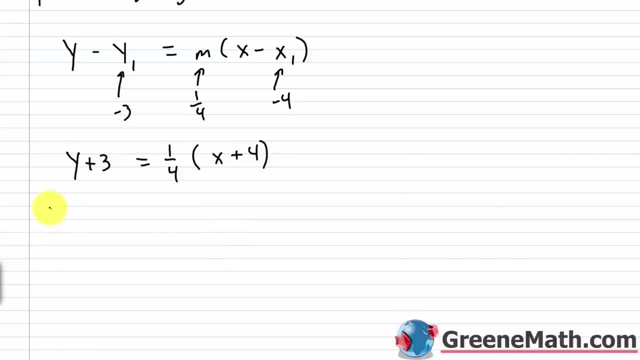 If it asked for that, we'd stop there. Solving it for y is pretty easy. We just have: y plus 3 is equal to 1 fourth times x is just 1 fourth x, so you can put x over 4,. 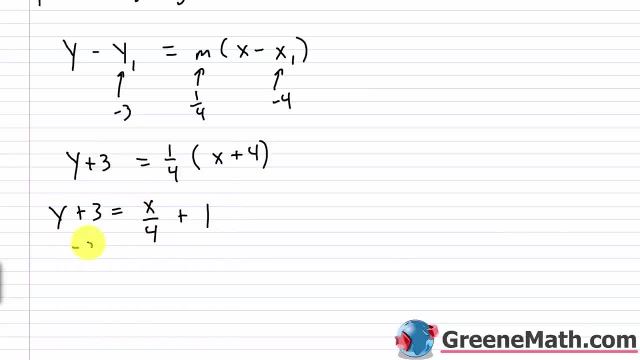 and then plus 1 fourth times 4 is 1.. So then I'd subtract 3 away from each side. I'll go ahead and just do this like this: y equals m times 3.. x over 4 plus, and basically it's gonna be negative 2.. 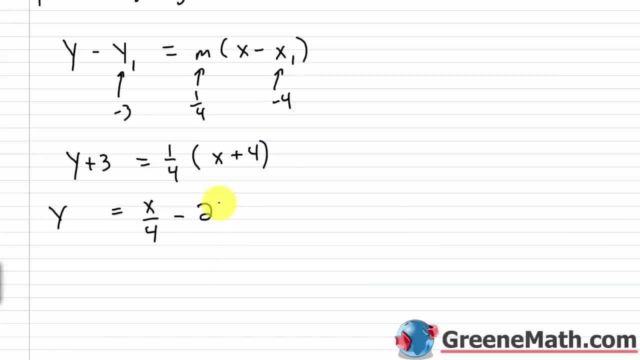 All right, you can put minus 2.. So now I have the equation in slope intercept form, y equals and you could write it as x over 4, or you could write 1 fourth times x minus 2.. It doesn't matter. 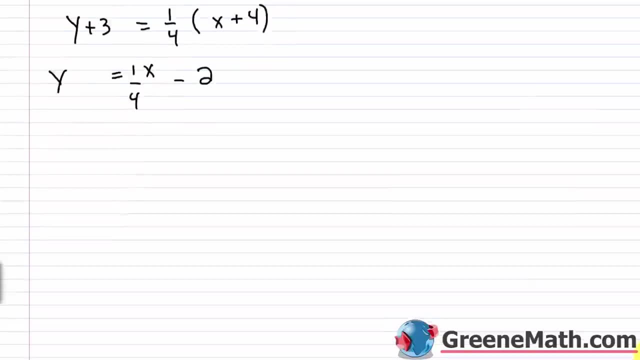 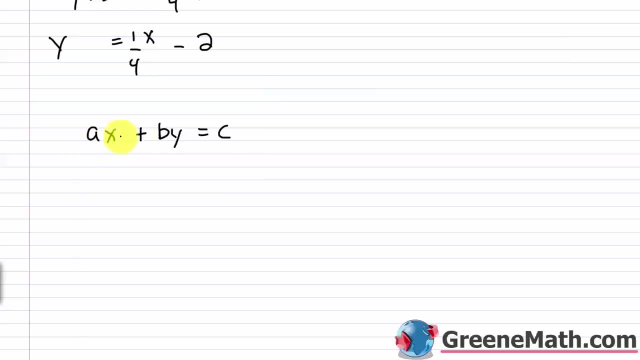 And I wanna put it in standard form. And again, let me kind of cover that definition again, Standard form looks like this: Ax plus by equals c, Again, where ab and c are equal to 1. So I'm gonna put that here. 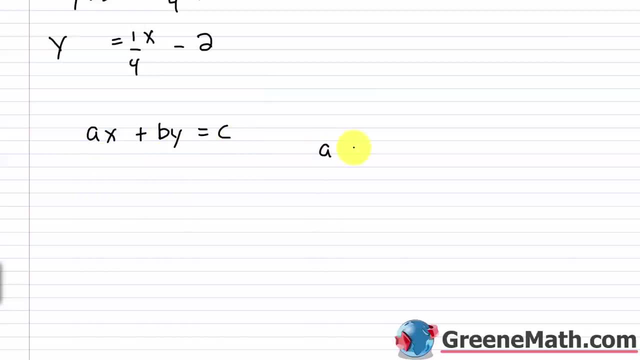 A and b are integers. A and b are not both 0. And a is greater than or equal to 0. Now what I wanna do? again, I have y equals 1, fourth x minus 2. I've kind of got two steps that I need to do. 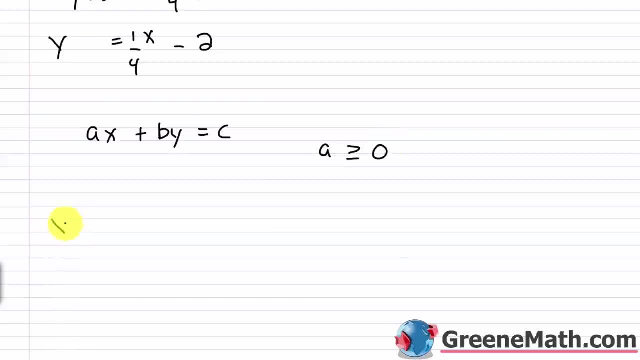 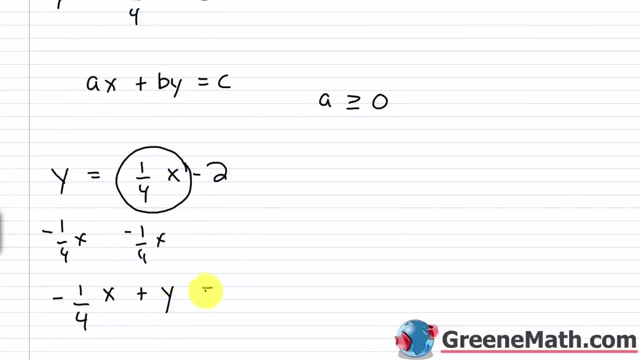 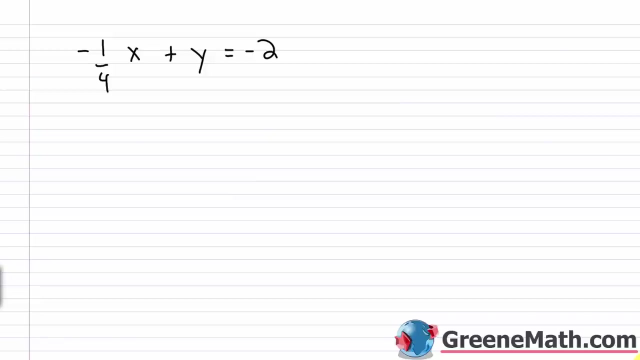 Now, what I want to do, again, I have y equals 1 fourth x minus 2. I've kind of got two steps that I need to do. I need to first start by subtracting this away from both sides of the equation. So if I do that, what's going to happen is I'm going to have negative 1 fourth x plus y is equal to negative 2. So once I've done that, again, we want a to be greater than or equal to 0, and we also want a, b, and c to be integers. So one of the things I can do is I can multiply by a negative, and that takes care of this being negative, right? It'll make it positive. But another thing I want to do, since I want integers, I want to clear this denominator of 4. So to do that, I would just multiply by 4, and if I'm multiplying by negative 1 and I'm multiplying by 4, I can combine those and just rule out the negative 1. So I'm going to do that, and I'm going to do that, and I'm multiplying by negative 1, and I'm multiplying by 4, and I can combine those, and just really multiply by negative 4, right? So I would multiply both sides of this equation by negative 4. And so negative 4 times negative 1 fourth, the negatives would cancel, and 4 over 4 is 1, so I'd basically just have x. And then plus, I have negative 4 times y, that's plus negative 4y, or I can just write minus 4y. And this equals negative 2 times negative 4, which is positive 8. 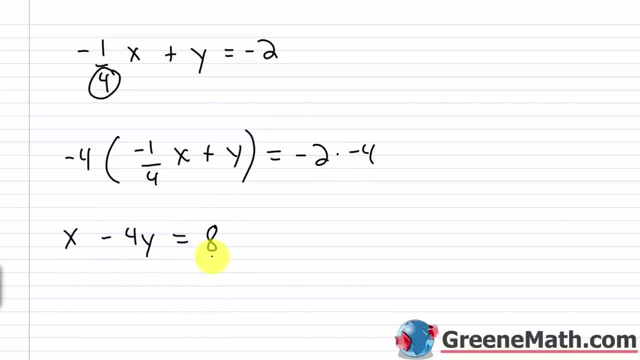 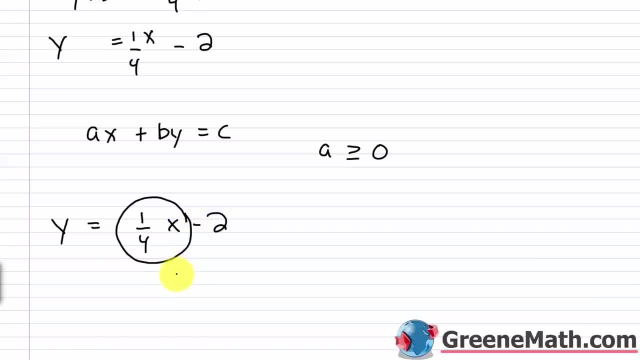 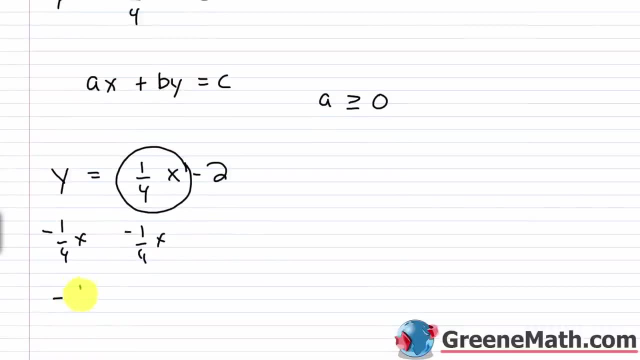 I need to first start by subtracting this away from both sides of the equation. So if I do that, what's gonna happen is I'm gonna have negative 1. fourth, x plus y is equal to negative 2.. So once I've done that, 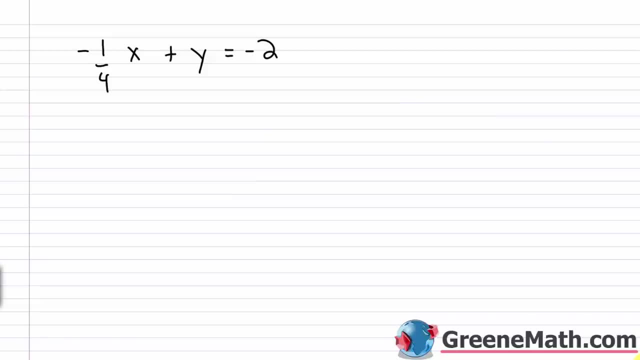 again, we want a to be greater than or equal to 0.. And we also want a, b and c to be integers. So one of the things I can do is I can multiply by a negative, and that takes care of this being negative. 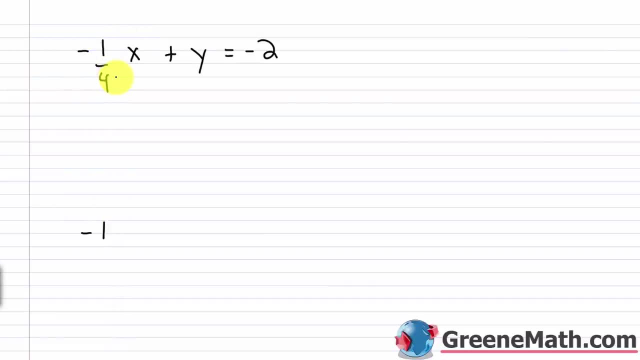 Right, it'll make it positive. But another thing I wanna do, since I want integers, I wanna clear this denominator of 4.. So to do that, I would just multiply by 4. And if I multiply by negative, 1,. 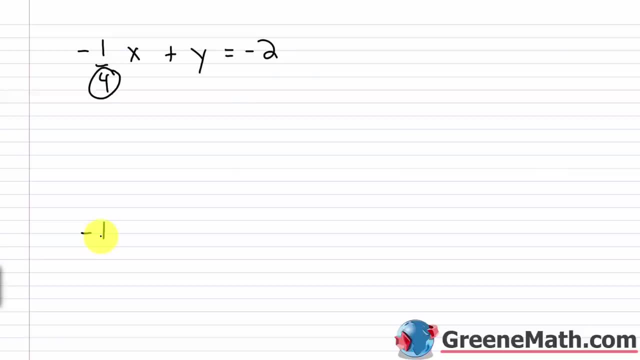 and I'm multiplying by 4, I can combine those and just really multiply by negative 4.. Right, so I would multiply both sides of this equation by negative 4.. And so negative 4 times negative 1. fourth, 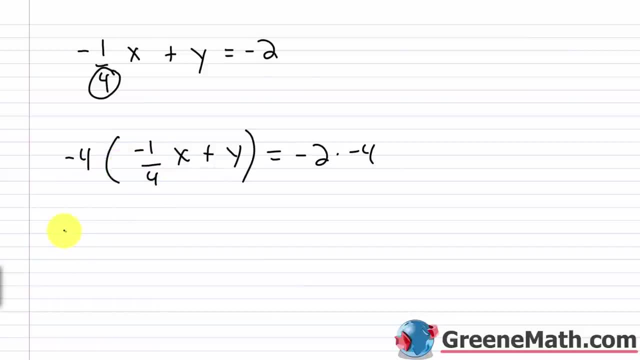 the negatives would cancel, and 4 over 4 is 1, so I'd basically just have x And then plus I have negative 4 times y. that's plus negative 4y, or I can just write minus 4y. 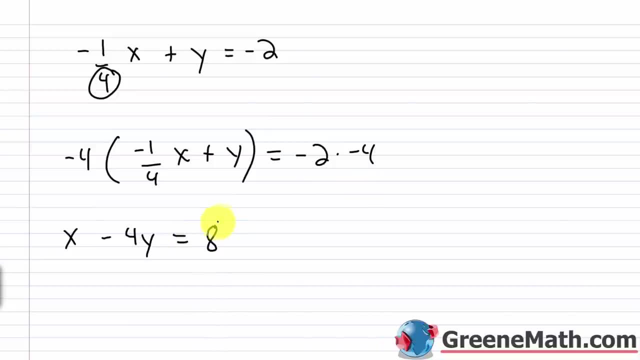 And this equals negative 2 times negative 4, which is positive 8.. So I have x minus 4y equals 8, and I'll fit the definition of standard form. I have ax plus by equals c, where a, which in this case is 1,. 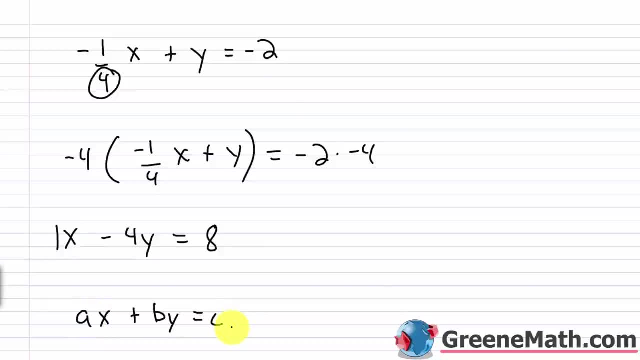 is greater than or equal to 0.. a, b and c are all integers, so I have a 1,, a negative 4, and an 8. That's perfectly fine. And then a and b are not both 0.. 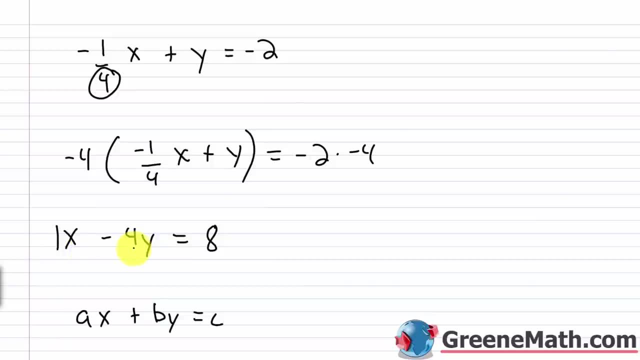 Neither are 0 in this case. so we're good to go. So we have x minus 4y equals 8, or again you could say: 1x minus 4y equals 8, as our, as our equation in standard form. 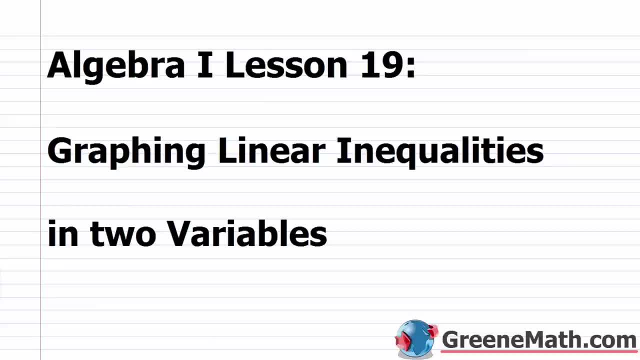 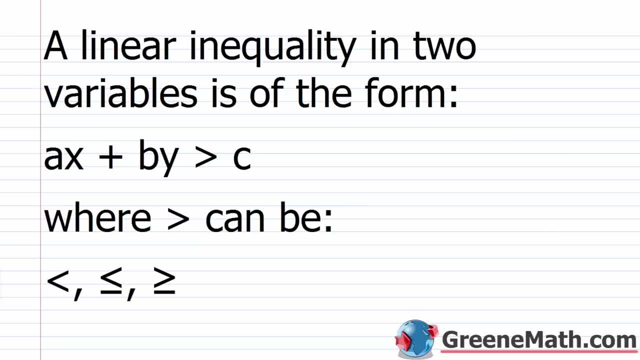 Hello and welcome to Algebra 1, lesson 19.. In this video we're going to learn about graphing linear inequalities in two variables. So a linear inequality in two variables is of the form: ax plus by is greater than c, where our greater than here can also be a less than. 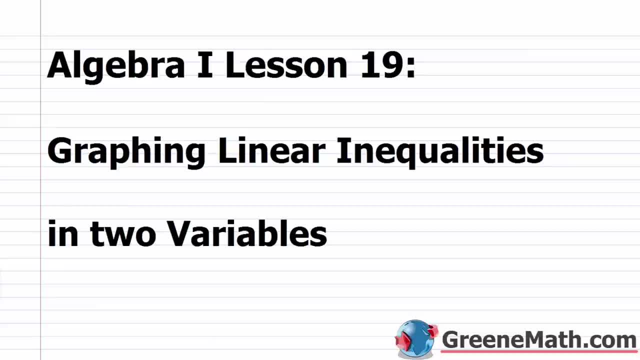 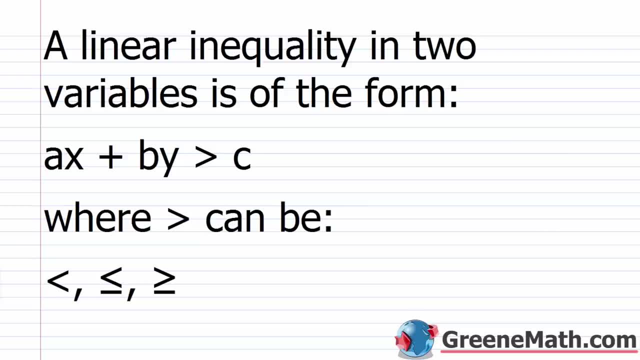 Hello, and welcome to Algebra 1, Lesson 19. In this video, we're going to learn about graphing linear inequalities in two variables. So a linear inequality in two variables is of the form ax plus by is greater than c, where our greater than here can also be a less than, a less than or equal to, or it can be a greater than or equal to. Now, some specific things about this form. 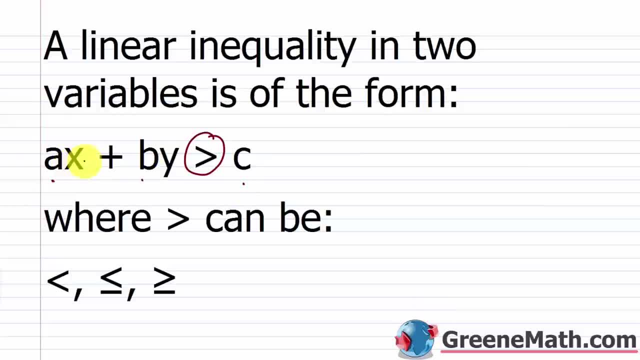 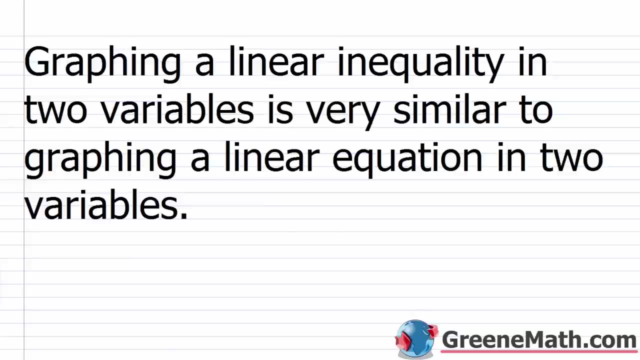 We have a, a b, and a c. a is a coefficient of x, b is a coefficient of y, and c, which is a constant. So a, b, and c are real numbers, and a and b cannot both be 0, meaning a could be 0, or b could be 0, but they can't both be 0 at the same time. All right, so graphing a linear inequality in two variables is very similar to graphing a linear equation in two variables. If you can graph a linear equation in two variables, you can get a linear equation in two variables. 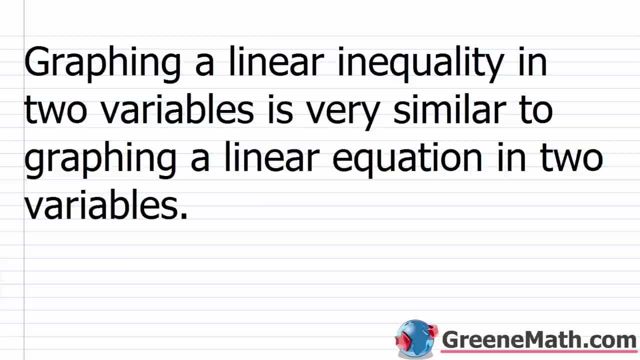 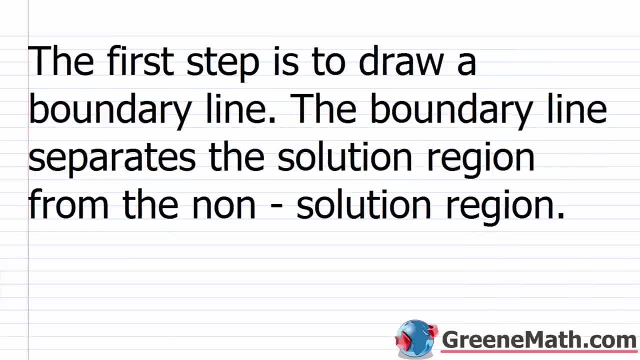 at this point, which you should be able to, then graphing a linear inequality in two variables is going to be no more difficult. There's really just one additional step. So the first thing that you 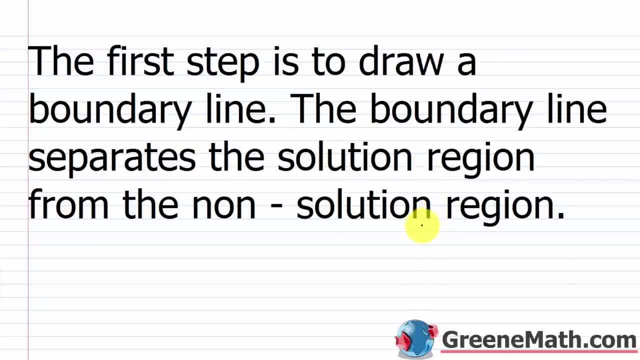 want to do is draw something known as a boundary line. So this is a very important concept for this topic, and we talked about it a little bit when we talked about checking our solution for a linear inequality in one variable. But the boundary line basically separates the solution from the non-solution region. So in other words, if I have a line, let's say it looks like this, and it's on my coordinate plane. Well, on one side of it, the ordered pairs or the points would work. Let's say this is my solution region. 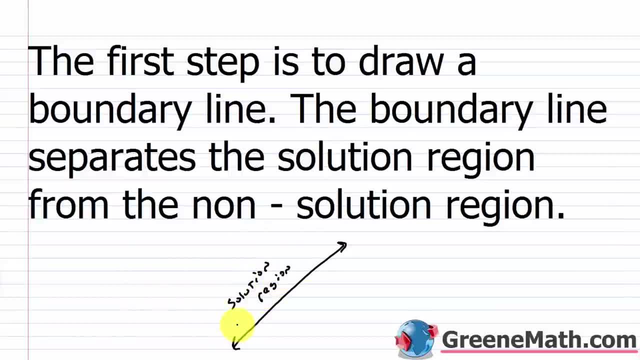 So if I take values from over here, ordered pairs, or you could say points, and I plug them into the 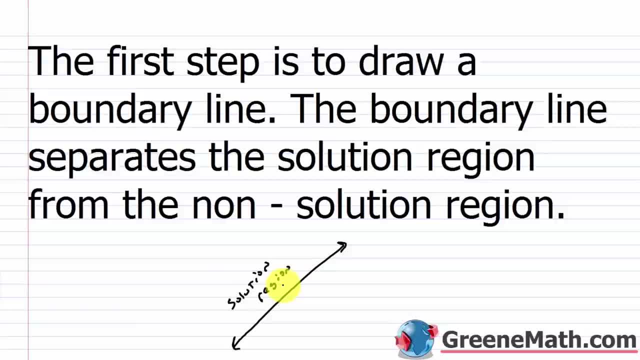 original inequality, I get a true statement. Then over here, let's say this is the non-solution region. 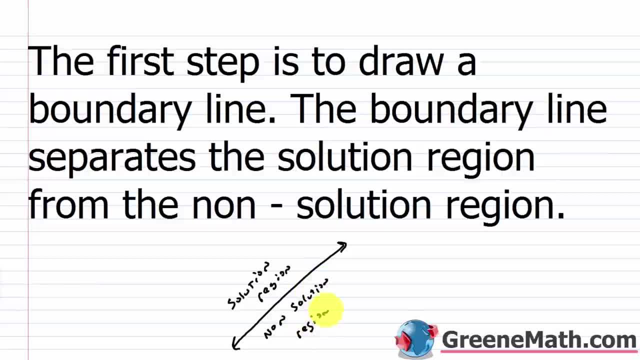 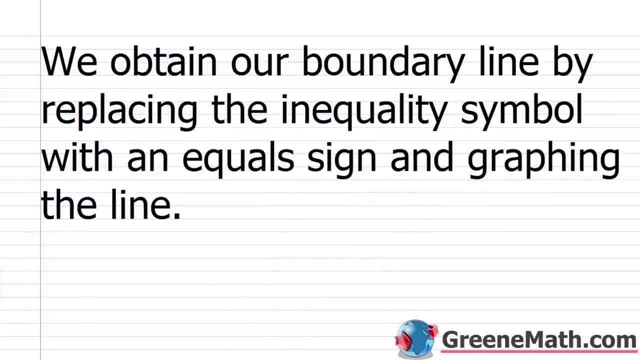 So ordered pairs or points over here are not going to work. So this line is what's going to separate the two. This is called, again, the boundary line, the boundary line. So we obtain our boundary line by replacing the inequality symbol with an equal sign and graphing the line. 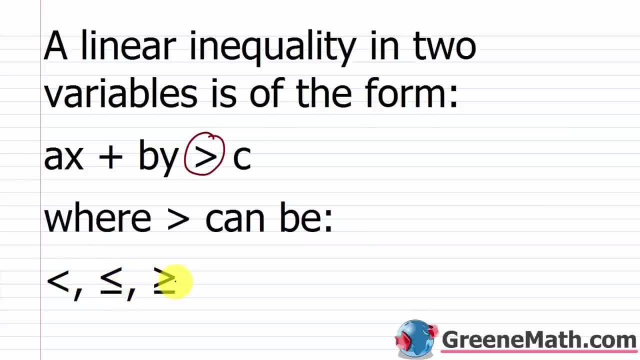 a less than or equal to, or it can be a greater than or equal to. Now some specific things about this form. We have a, a, b to c. a is a coefficient of x, b is a coefficient of y and c, which is a constant. So a, b and c. 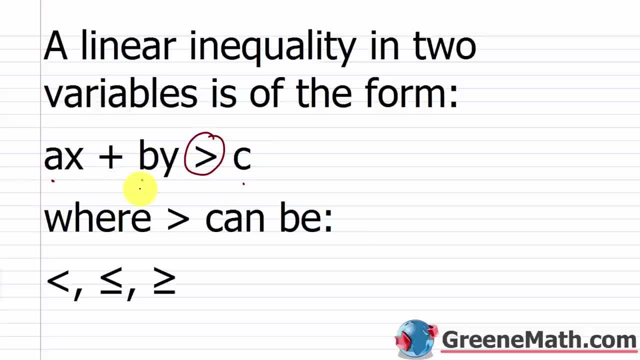 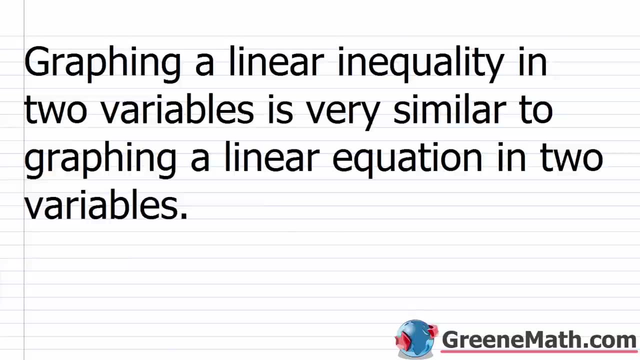 are real numbers and a and b cannot both be zero. meaning a could be zero or b could be zero, but they can't both be zero at the same time. All right, so graphing a linear inequality in two variables is very similar to graphing a linear equation in two variables. If you can graph a, 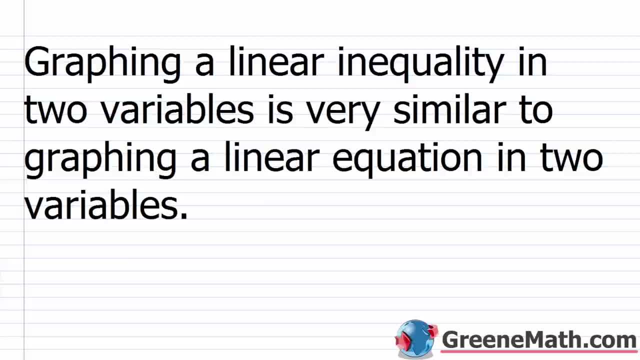 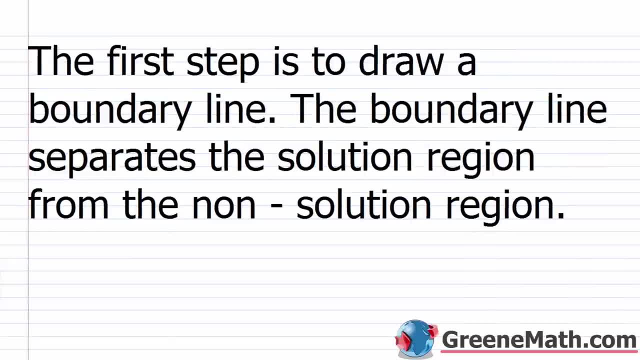 linear equation in two variables at this point, which you should be able to, then graphing a linear inequality in two variables is going to be no more difficult. There's really just one additional step, So the first thing that you want to do is draw something known as a boundary line. 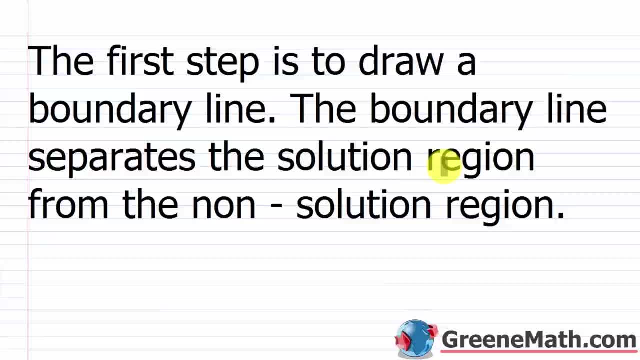 So this is a very important concept for this topic and we talked about it a little bit when we talked about checking our solution for a linear inequality in one variable. But the boundary line basically separates the solution response from the solution response from the solution response. 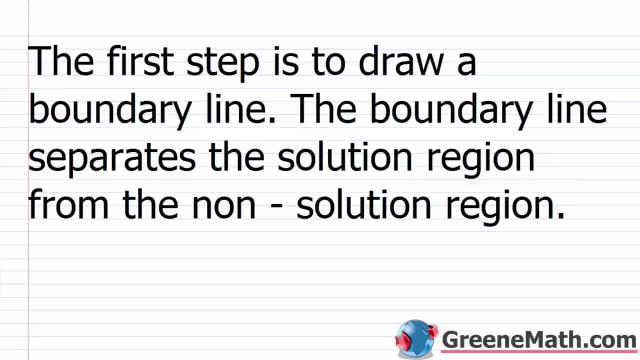 So the boundary line separates the solution response from the solution response from the non-solution region. So in other words, if I have a line- let's say it looks like this and it's on my coordinate plane- Well, on one side of it the ordered pairs or the points would work. Let's say this is my. 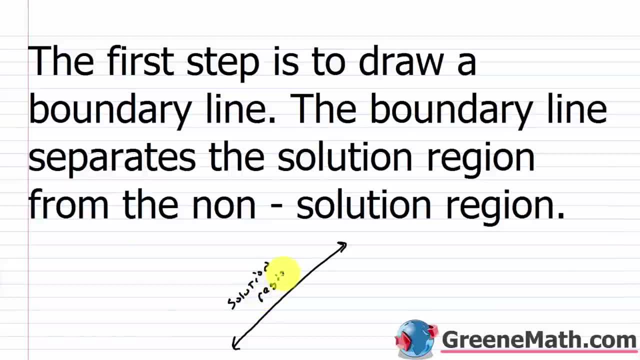 solution region. So if I take values from over here- ordered pairs, or you could say points, and I plug them into the original inequality, I get a true statement. Then over here let's say: this is the non-solution region. So if I take values from over here- ordered pairs, or you could say points: 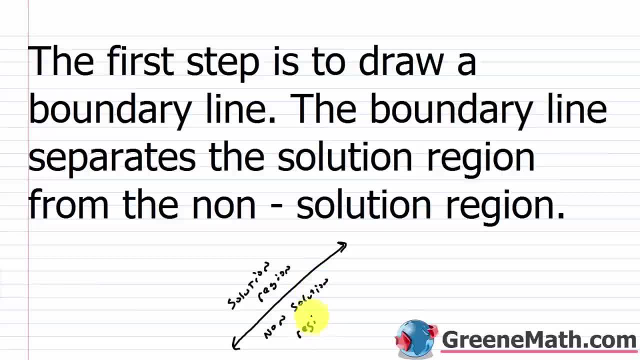 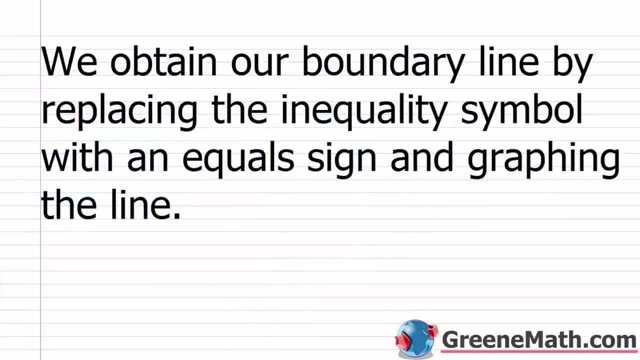 over here are not going to work. So this line is what's going to separate the two. This is called again the boundary line, The boundary line. So we obtain our boundary line by replacing the inequality symbol with an equal sign and graphing the line. So, essentially, all you're doing is 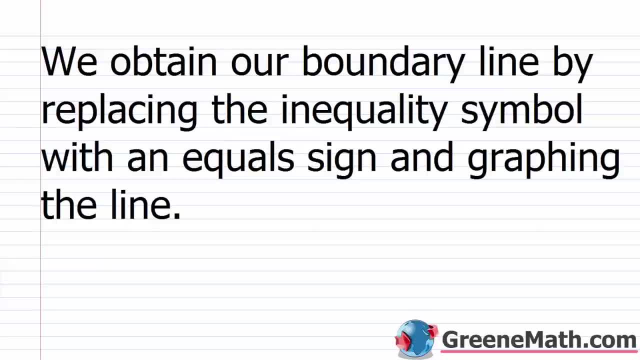 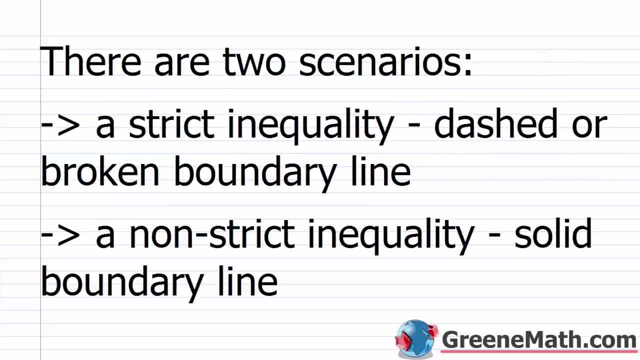 starting out by taking your linear inequality in two variables and transforming it into a linear inequality in two variables and just graphing it. But there's one thing you really need to know before you do that. So there's two scenarios. So a strict inequality, So strictly less than or. 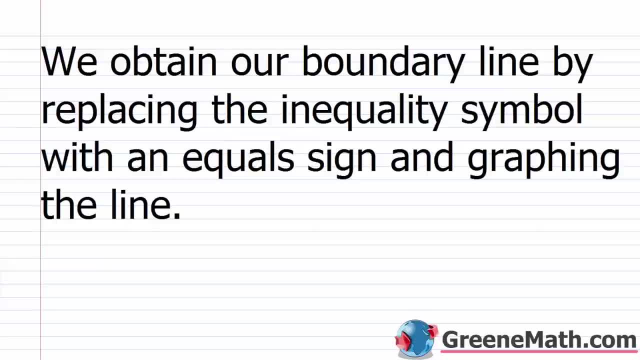 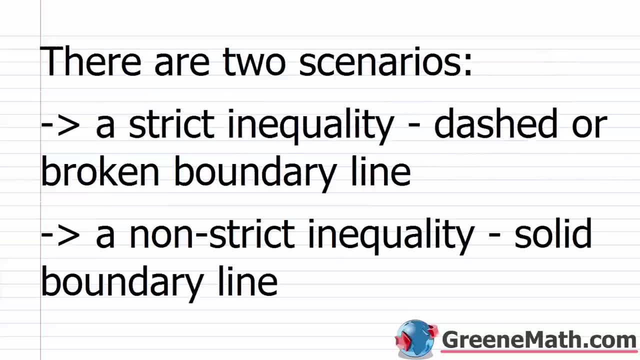 So essentially, all you're doing is you're starting out by taking your linear inequality in two variables and transforming it into a linear equation. But there's one thing you really need to know before you do that. So there's two scenarios. 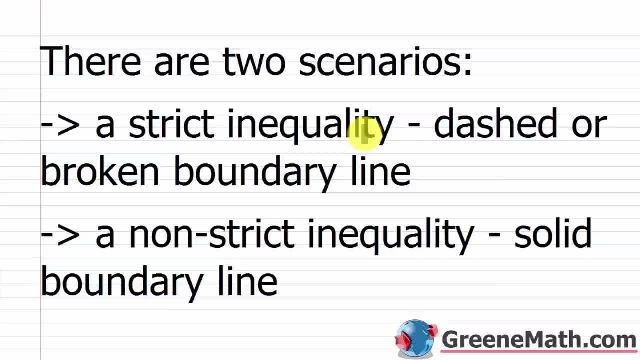 So a strict inequality, so strictly less than or strictly greater than, 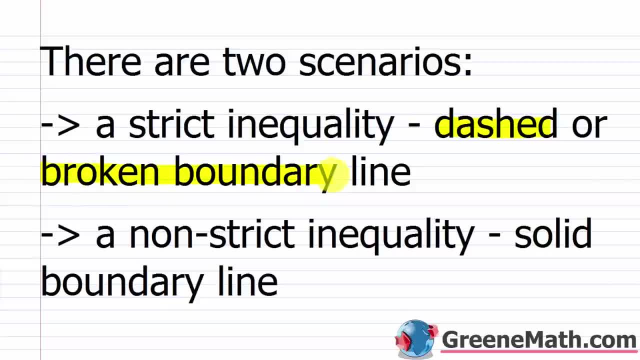 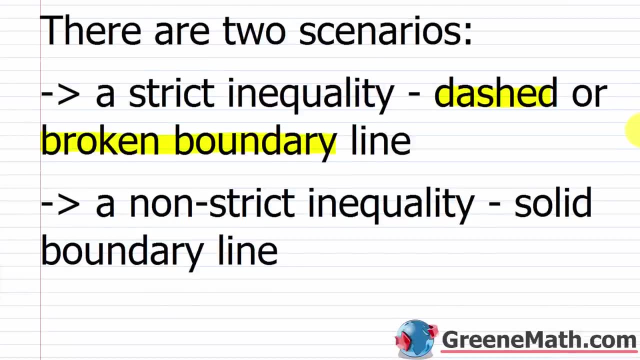 that gives us a dashed or broken boundary line. And why do you think that is? Well, if you have a strict inequality, the boundary line is not part of your solution. And I want you to recall at this point when we talked about a linear inequality in one variable. Let's say I saw something like x is less than 3. This was strict. So we had notation when we graphed this on the number line. So let's say this is 0. This is 1, 2, 3, 4. Let's say over here, this is negative 1, negative 2, negative 3, negative 4. So when we graphed x is less than 3, we found 3, and we said 3 is not included. So what we did was we put a parenthesis there facing to the left. I know some of you put an open circle, but it's the same thing. And then we shaded everything to the left. 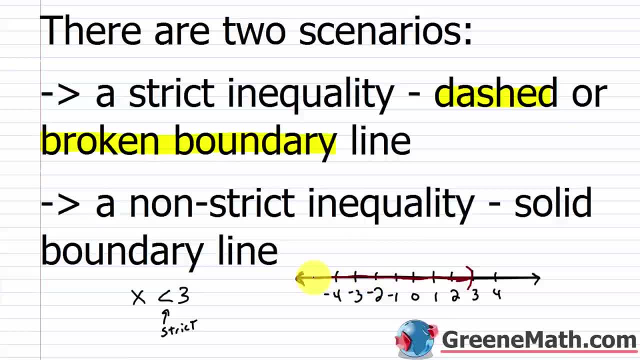 So this is very similar. When we use a dashed or broken boundary line, it's kind of like the parenthesis was here. We're saying it's not included as part of the solution. 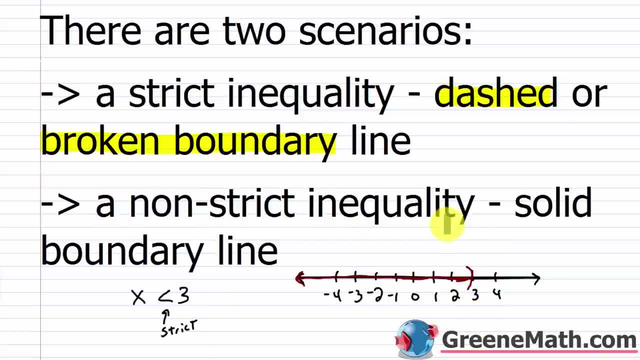 So then kind of the next scenario would be a non-strict inequality. 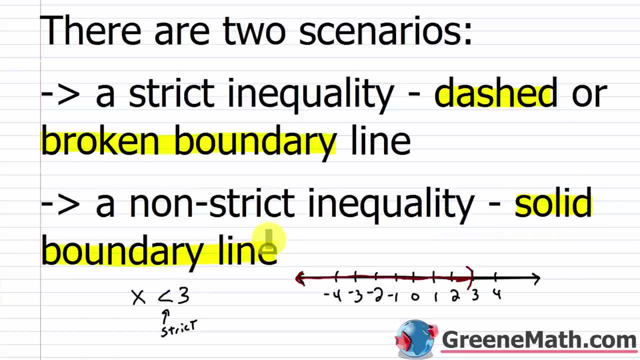 And for that, we're going to use a dashed or broken boundary line. And for that, we're going to use a dashed or broken boundary line. And for that, we're going to use a dashed or broken boundary line. And for this one, you're going to have a solid boundary line, a solid boundary line. 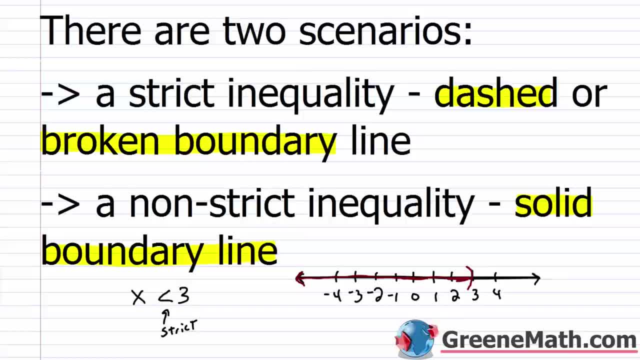 And the reason for that is it's included. So let's say I had something like x is less than or now equal to 3. Instead of the parenthesis, I had a bracket. So it's similar to that because the bracket told me that 3 was included. So that's what we're doing here with the solid boundary 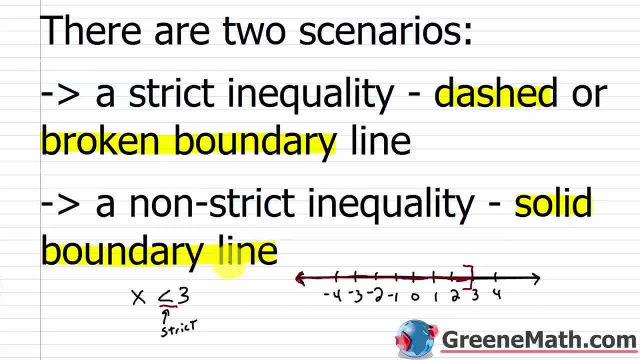 line. That line is included as part of the solution. All right, so let's start out with 2x plus y is less than or equal to 1. 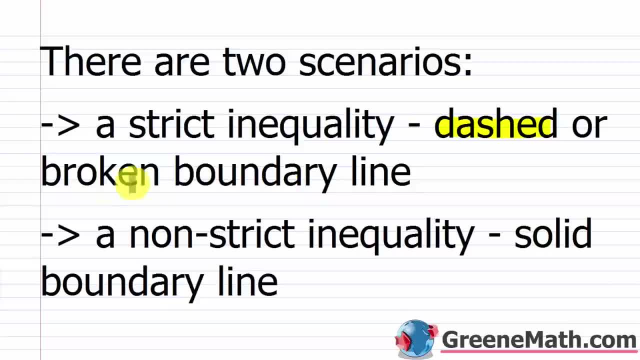 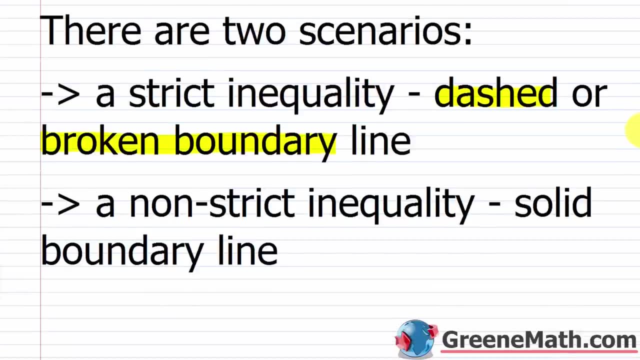 strictly greater than That gives us a dashed or broken boundary line. And why do you think that is? Well, if you have a strict inequality, the boundary line is not part of your solution, And I want you to recall at this point when we talked about a linear inequality in one variable. 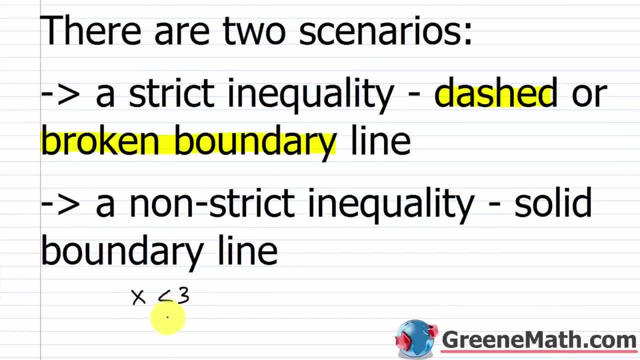 Let's say, I saw something like x is less than 3.. This was strict, So we had notation when we graphed this on the number line. So let's say this is 0.. This is 1,, 2,, 3,, 4.. Let's say, over here, this is: 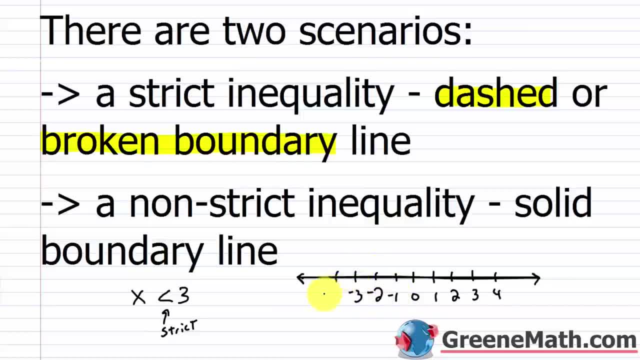 negative 1, negative 2, negative 3, negative 4.. So when we graphed x is less than 3, we found 3 and we said 3 is not included. So what we did was we put a parenthesis there, facing to the left. I know some of you put an open circle, but 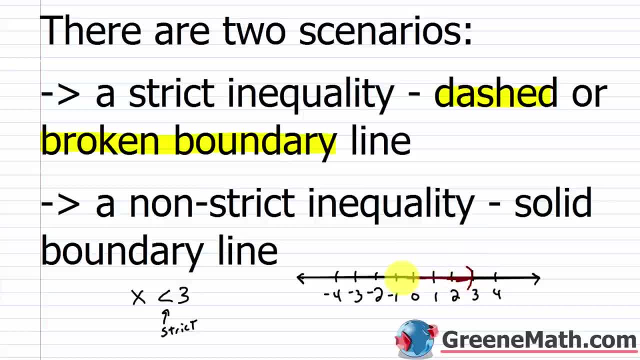 it's the same thing, And then we shaded everything to the left. So this is very similar When we use a dashed or broken boundary line. it's kind of like the parenthesis was here. We're saying it's not included as part of the solution, So then kind. 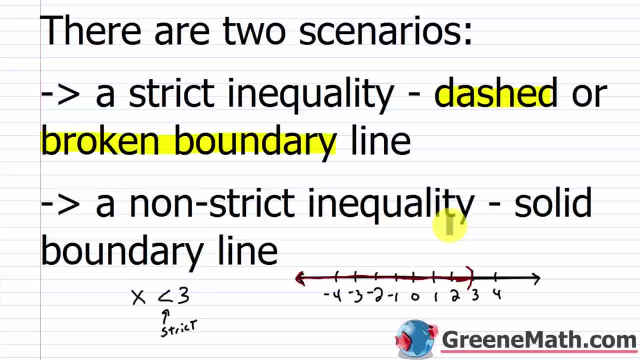 of the next scenario would be a non-strict inequality, And for this one you're going to have a solid boundary line, A solid boundary line, And the reason for that is it's included. So let's say, I had something like x is less than or now equal. 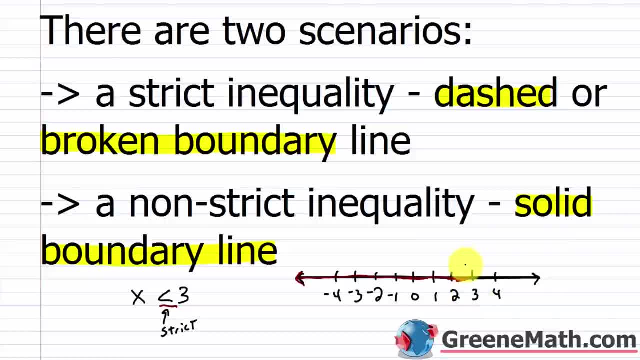 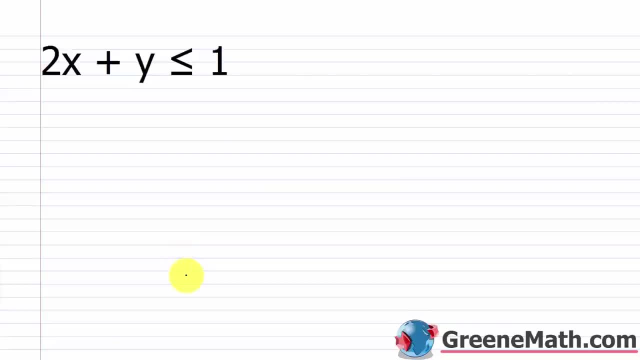 to 3.. Instead of the parenthesis, I had a bracket, So it's similar to that, because the bracket told me that 3 was included. So that's what we're doing here with the solid boundary line. That line is included as part of the solution. All right, so let's start out with. 2x plus y is less than or. 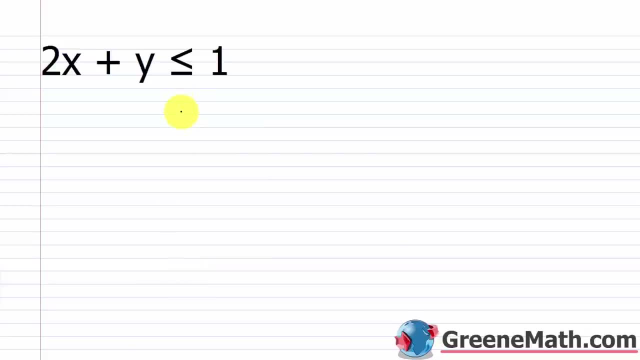 equal to 1.. So I'm going to do this the slow way to start. I'm going to put an equal sign here. I'm going to put 2x plus y equals 1.. I'm going to graph it the slow way. So I'm going to make some ordered pairs. 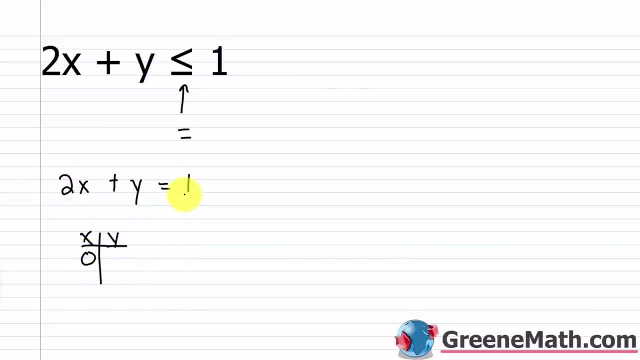 And I can see immediately: if I put a 0 in for x, y would be 1.. That's the y intercept. That's easy. And then to get some other points going, I can't put a 0 in for y, because if I do I'm not going. 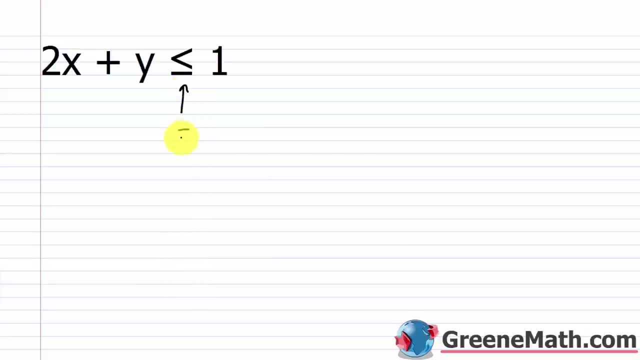 So I'm going to do this the slow way to start. I'm going to put an equal sign here. I'm going to put 2x plus y equals 1. I'm going to graph it the slow way. So I'm going to make some ordered pairs. 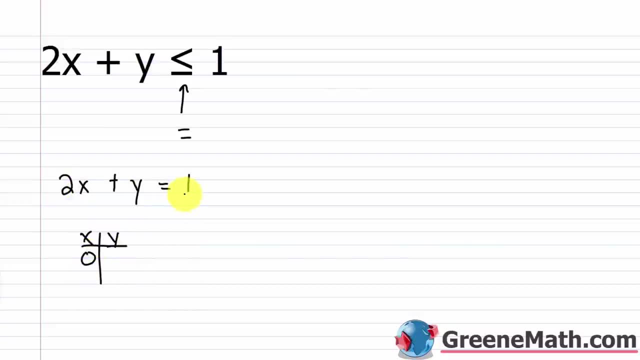 And I can see immediately if I put a 0 in for x, y would be 1. That's the y-intercept. That's easy. 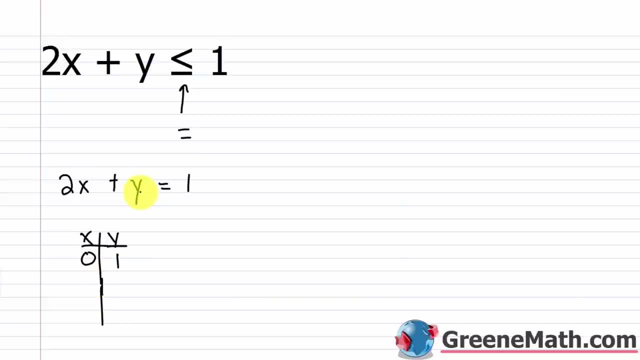 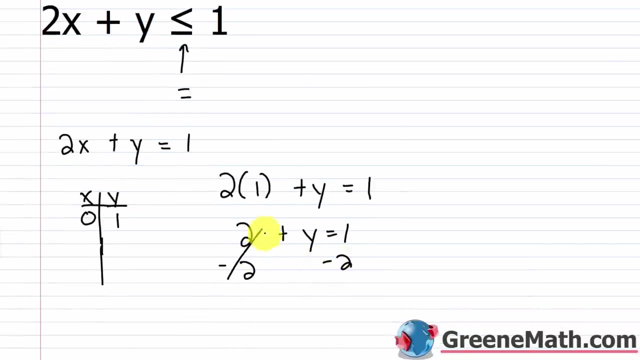 And then to get some other points going, I can't put a 0 in for y because if I do, I'm not going to end up with an integer. I'd plug in a 0 for y. You'd end up with x equals 1 half. So that's not something that I want to deal with on my coordinate plane. So let's try if x was 1. So 2 times 1 plus y equals 1. So this would be 2 plus y equals 1. And so subtract 2 from both sides of the equation. That's gone. I'd have y is equal to negative 1. So if x is 1, y is negative 1. And let's try a value of x equals 2. 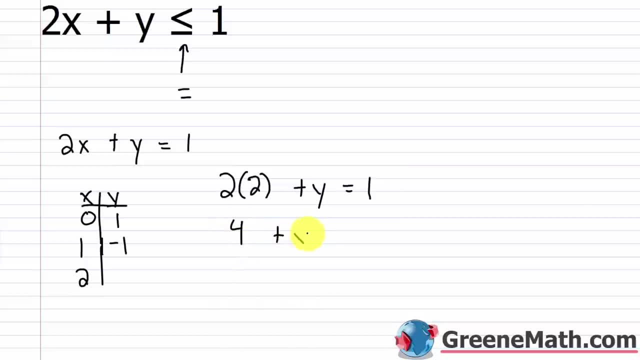 So if x is 2, this would be 4 plus y equals 1. 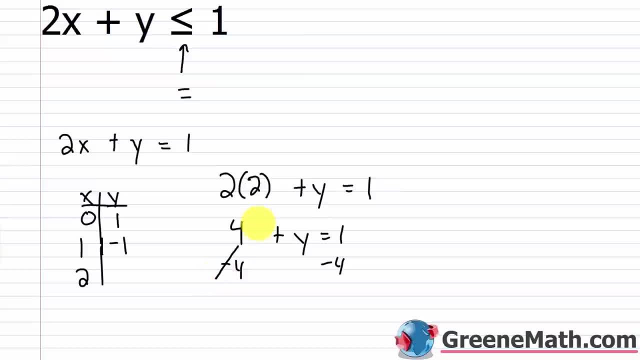 Y equals 1. Subtract 4 from each side of the equation. That's gone. Y is equal to negative 3. All right. So I have three ordered pairs. Let's plot those ordered 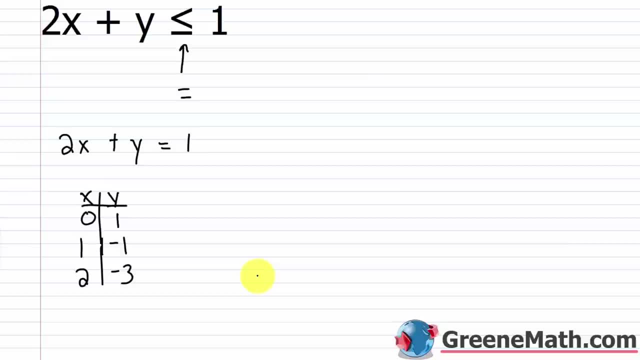 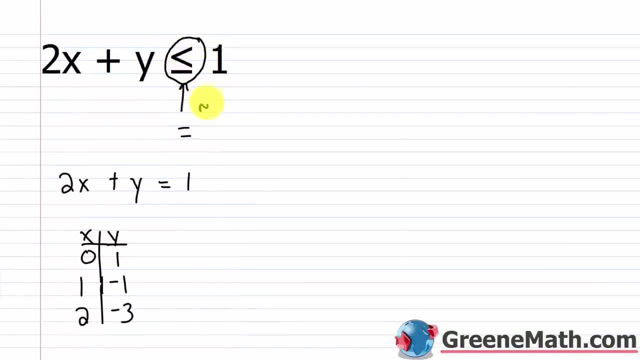 pairs. And let's draw a line. This line is going to be our boundary line. Now what do we want? We have a non-strict inequality. This is non-strict. So if we have a non-strict inequality, the boundary line is part of the solution. So 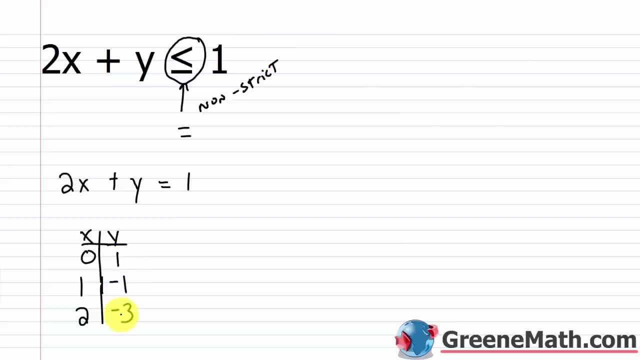 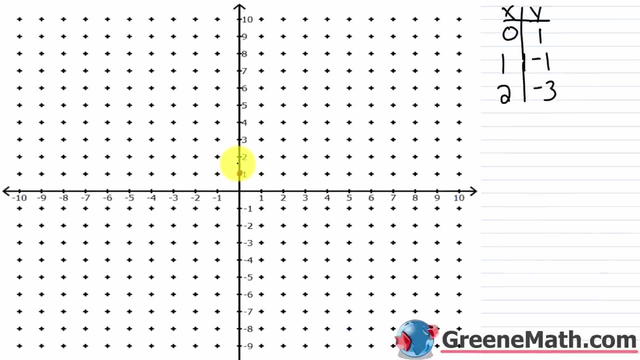 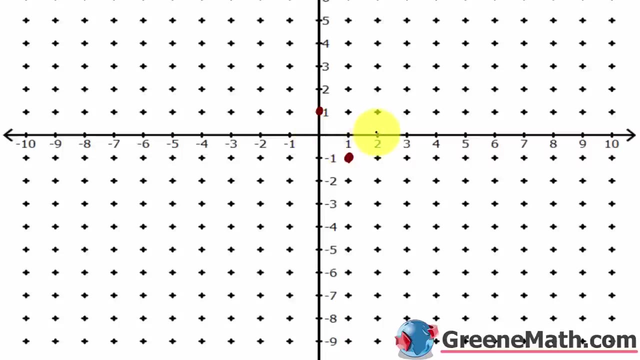 we want a solid line. So let's go draw a solid line. So I want the point 0 comma 1. That's right here. I want the point 1 comma negative 1. That's going to be right here. And I want the point 2 comma negative 3. So 2 over to the right, 3 down. That's right there. And again, we're going to draw a solid line. 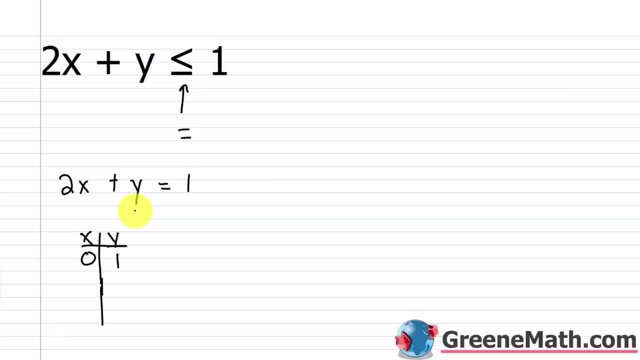 to end up with an integer. I'd plug in a 0 for y. You'd end up with a 0 for y. So I'm going to write: 2x plus y equals 1.. So that's not something that I want to deal with on my coordinate plane. 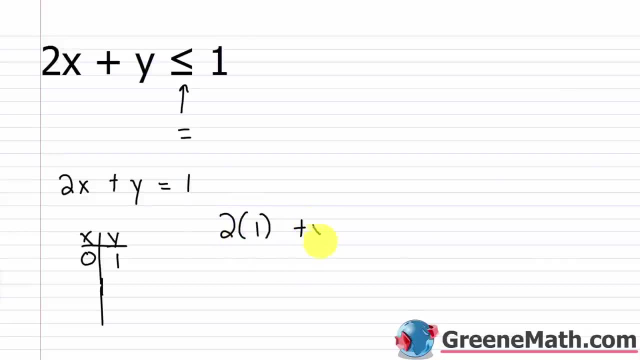 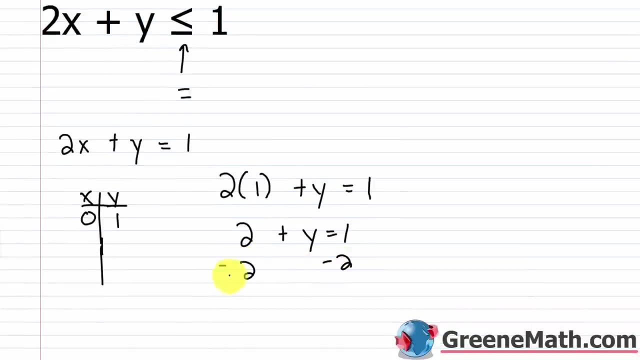 So let's try. if x was 1.. So 2 times 1 plus y equals 1.. So this would be: 2 plus y equals 1.. And so subtract 2 from both sides of the equation That's gone. I'd have y is equal to negative 1.. 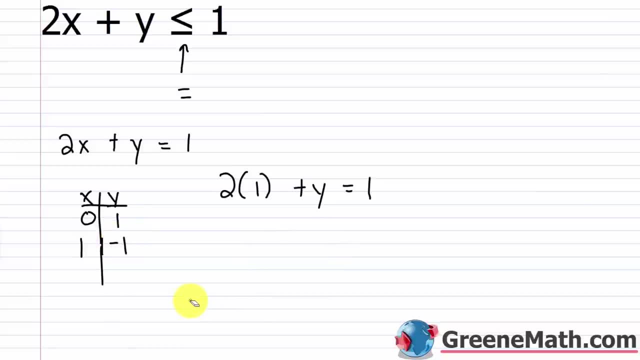 So if x is 1, y is negative 1. And let's try a value of x equals 2.. So if x is 2, this would be 4 plus y equals 1. Subtract 4 from each side of the equation, That's gone. y is equal to negative 3.. 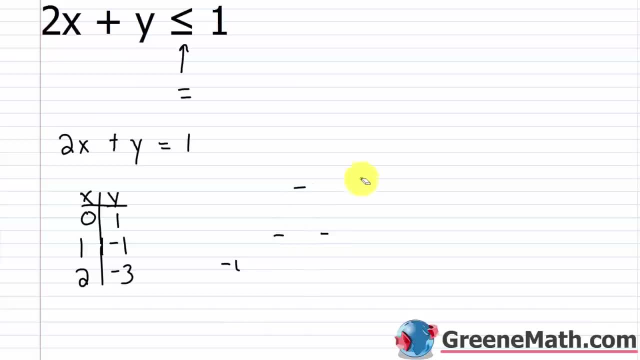 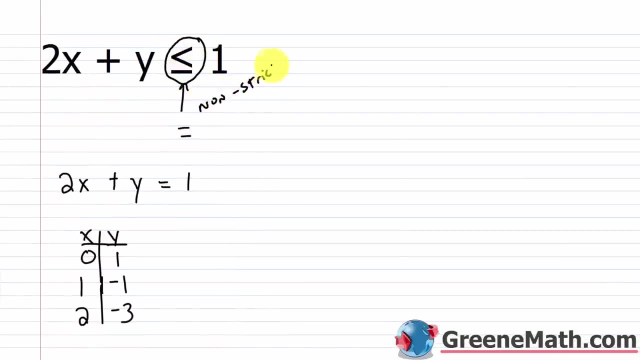 All right, So I have three ordered pairs. Let's plot those ordered pairs and let's draw a line. This line is going to be our boundary line. Now, what do we want? We have a non-strict inequality. This is non-strict. So if we have a non-strict inequality, the boundary line is part of the. 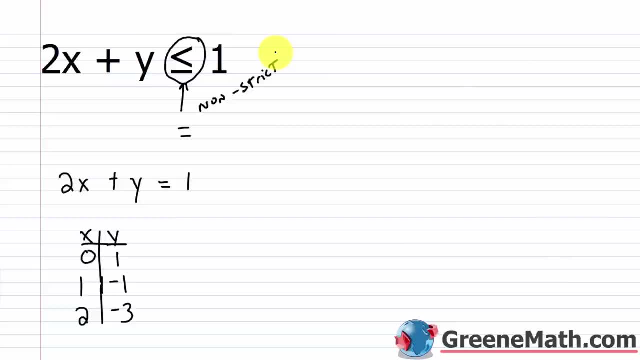 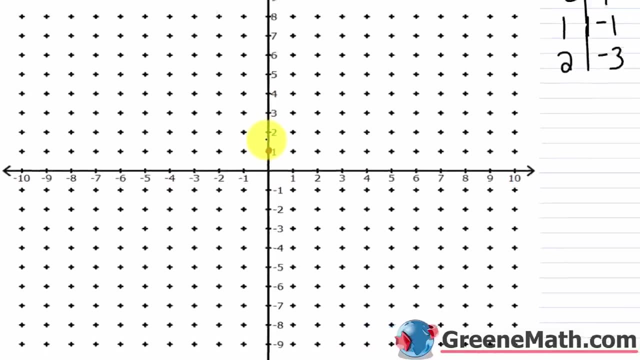 solution. So we want a solid line. So we want a non-strict inequality. So we want a non-strict line. so let's go draw a solid line. so I want the point 0 comma 1, that's right here. I want the point 1 comma negative 1, that's gonna be right here. and I want 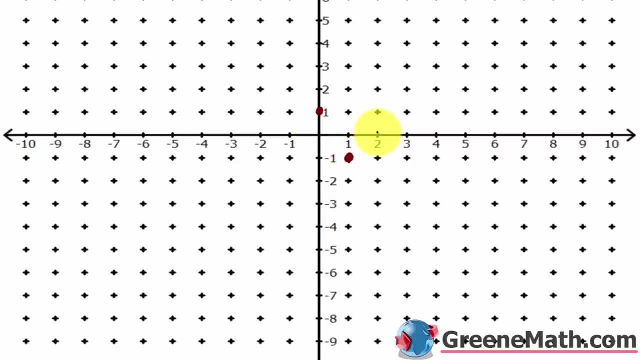 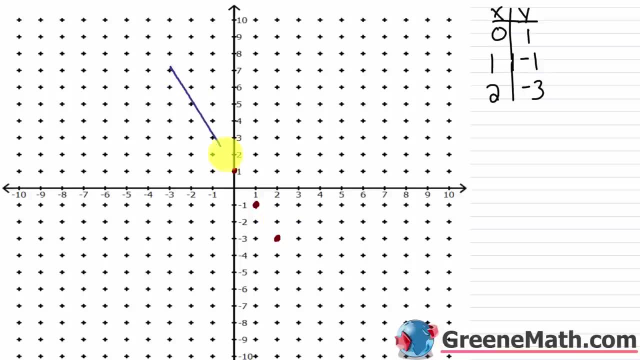 the point 2, comma, negative 3. so 2 over to the right, 3 down. that's right there, and again, we're gonna draw a solid line, okay? so once you've graphed the line, go back up to the top. now this is your one. 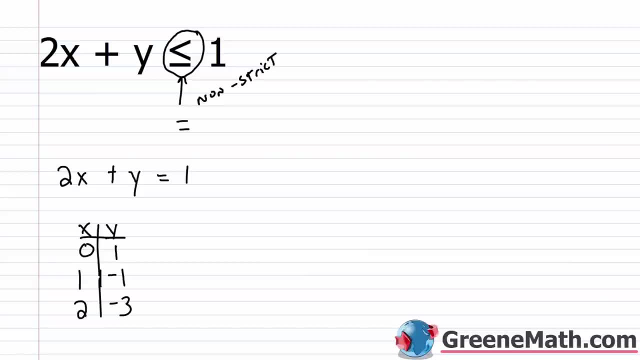 additional step. you're gonna read in your book something about a test point. a test point, okay, and the test point works like this: you can test any point on either side of the line. if it works, that means that side of the line is the solution region and therefore you're gonna shade that side of the line if it. 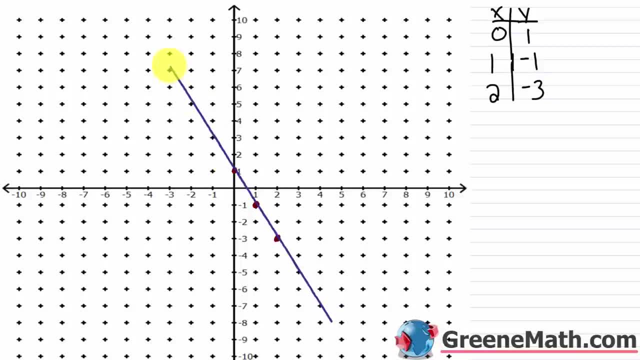 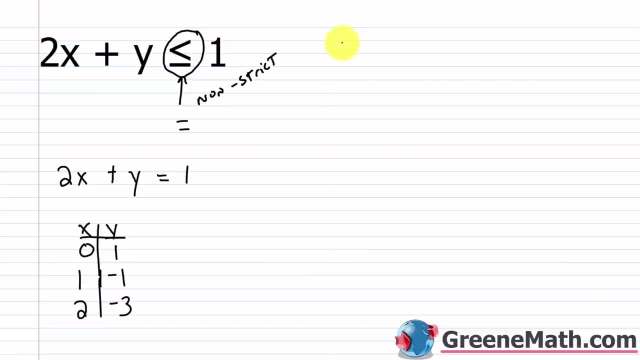 So let's draw a line. Okay. So once you've graphed the line, go back up to the top now. This is your one additional step. You're going to read in your book something about a test point. A test point. Okay. And the test point works like this. You can test any point on either side of the line. If it works, that means that side of the line is the solution region. And therefore, you're going to shade that side of the line. So that's the solution region. So now I want that side of the line, 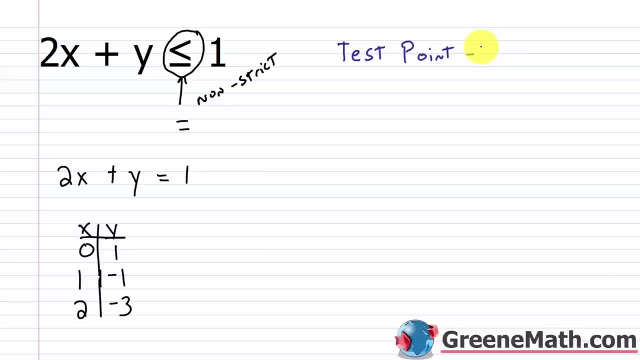 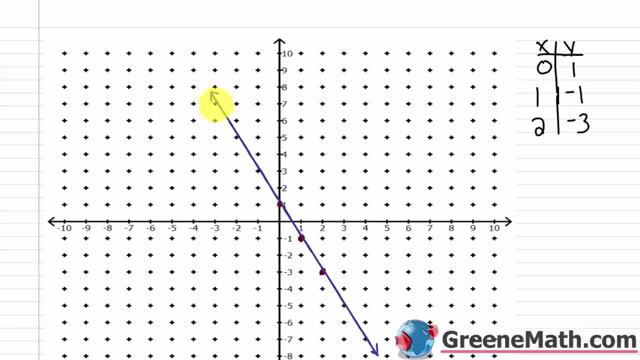 side of the line if it doesn't work you're in the non-solution region and you're going to shade the other side of the line so let's go back down here we look at we're not going to choose any point on the line because we already know that that's going to work as a solution the easiest point to choose 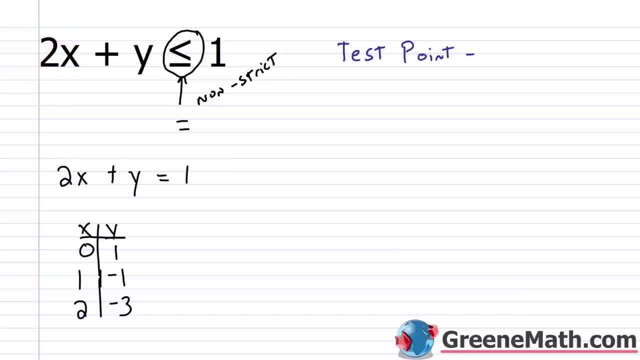 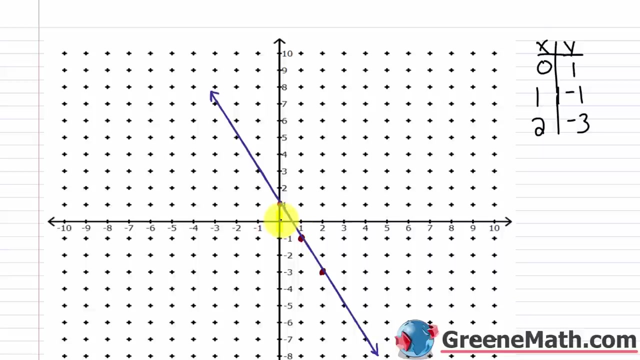 up and we're going to plug in a zero for x and a zero for y so my test point is zero comma zero so I would have two times zero plus zero is less than or equal to one so two times zero is zero plus zero is zero so zero is less than or equal to one that's true so what that tells me is that this point right here zero comma zero is on the solution region 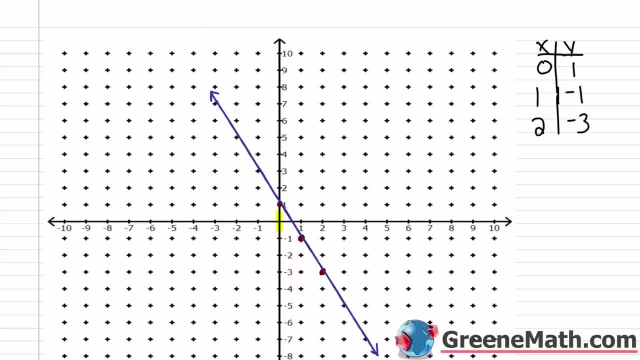 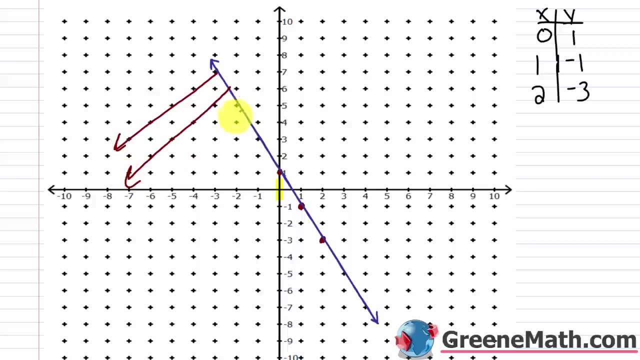 so that means that the solution region is below the line so you In other words, I would shade everything below the line, and it's hard to do a good job of shading, so I just kind of do it this way. 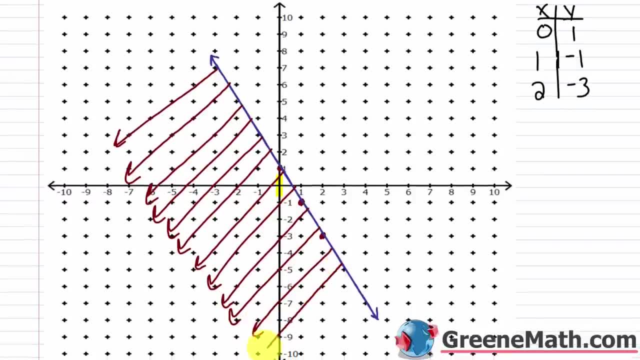 I know there's some computer programs that will shade this perfectly, but if you're doing this freehand, it's about as good as we're going to do. 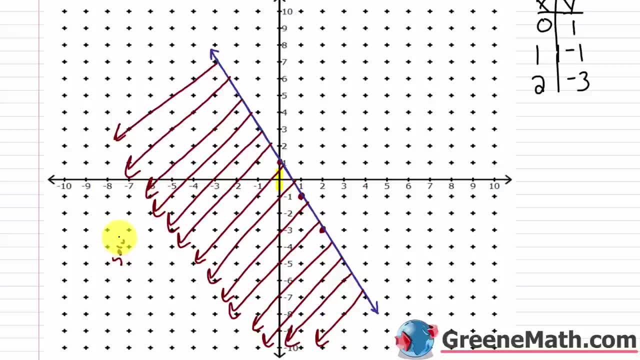 Okay, so in other words, this is the solution region. 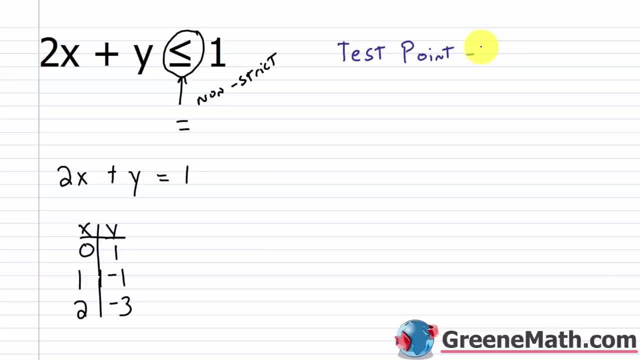 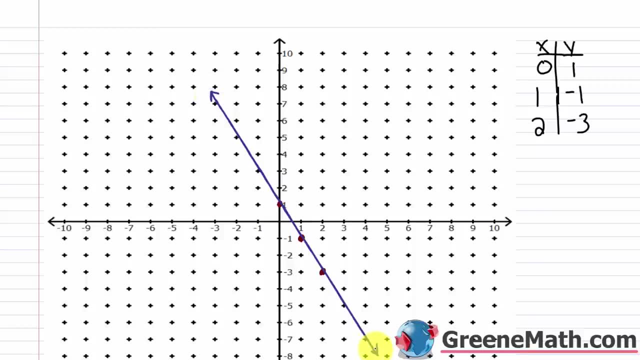 doesn't work. you're in the non solution region and you're going to shade the other side of the line. so let's go back down here we look at. we're not going to choose any point on the line because we already know that that's going to work. 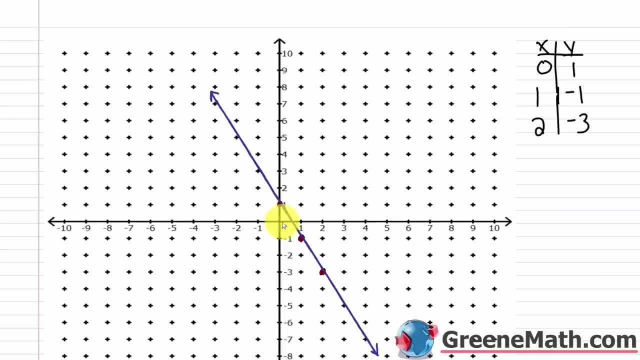 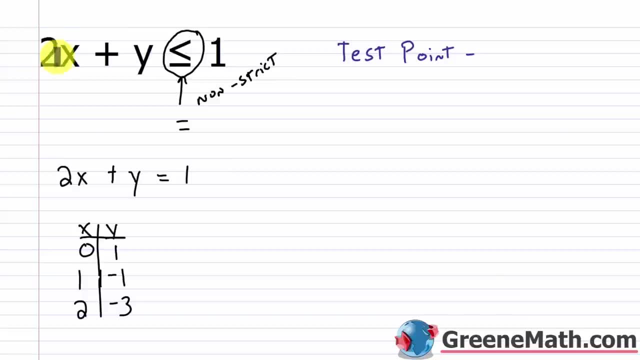 as a solution. the easiest point to choose, if it's not on your line, is 0 comma 0 right, because 0 is easy to find, and if it's not on your line, it's going to work as a solution easy to work with. so let's go back up and we're gonna plug in a 0 for X and a 0. 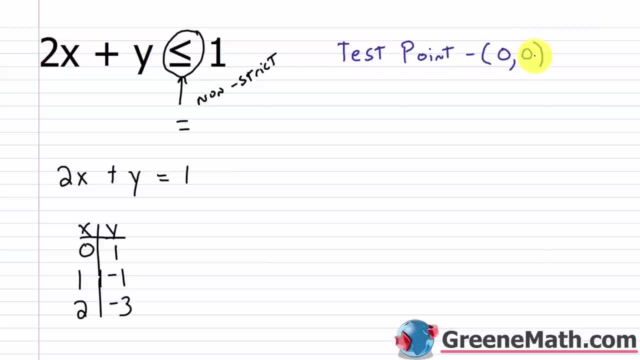 for Y, so my test point is 0 comma 0, so I would have: 2 times 0 plus 0 is less than or equal to 1, so 2 times 0 is 0 plus 0 is 0, so 0 is less than or equal to 1. 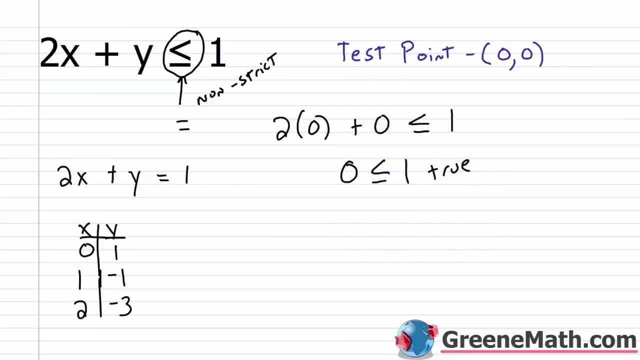 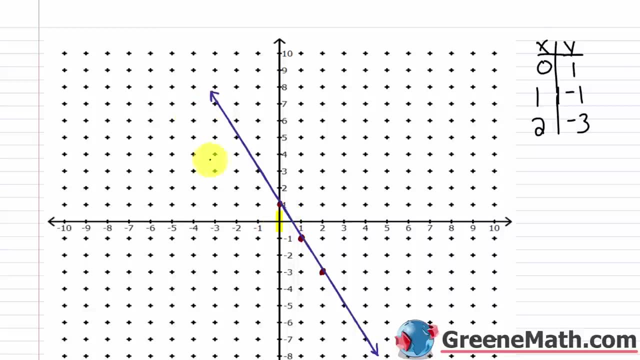 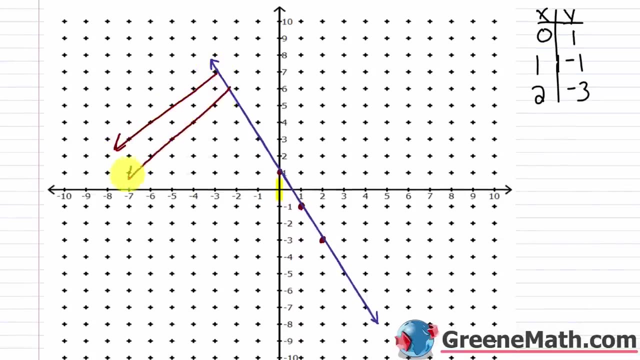 that's true. so what that tells me is that this point right here, 0 comma 0, is on the solution region. so that means that the solution region is below the line. so in other words, I would shade everything below the line, and it's hard to do a good job of shading, so I just kind of do it this way. 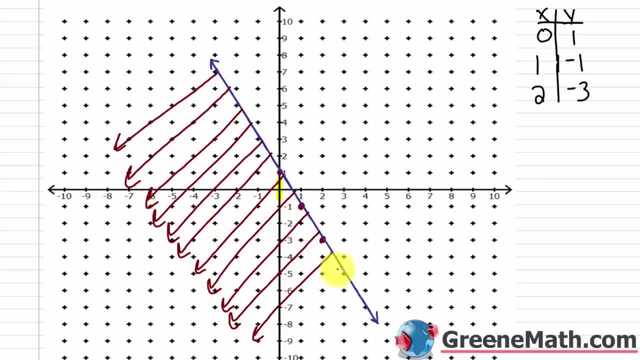 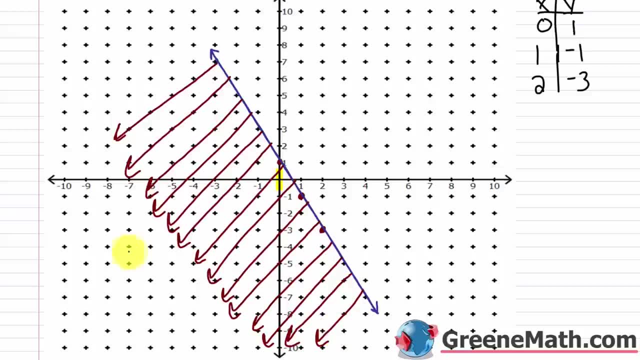 I know there's some computer programs that will shade this perfectly, but you're doing this freehand. it's about as good as we're gonna do, okay. so in other words, this is the solution region, but it's not going to work as a solution. so this is. 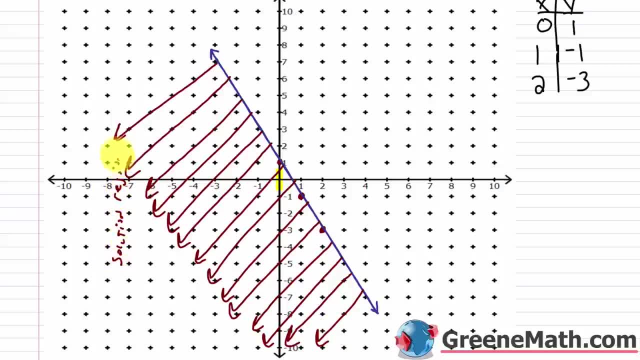 solution region, And over here anything kind of above this line is the non-solution, non-solution region. And just try it out for yourself. Pick some points over here. Pick six comma zero, for example. That is in the non-solution region. so it shouldn't work. 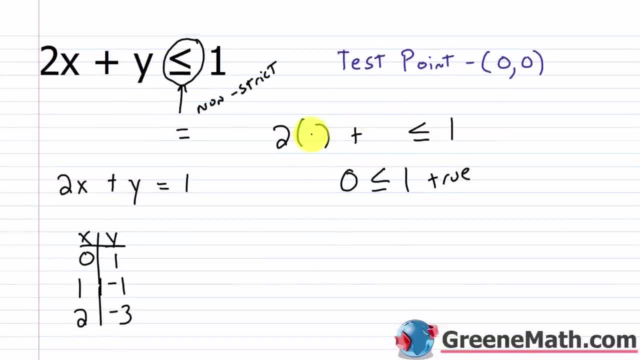 If I plug it in, I should get a false statement. So if I plug in a six for x and a zero for y, I should get a false statement. Two times six is 12, 12 plus zero is not going to be less than or equal to one right. 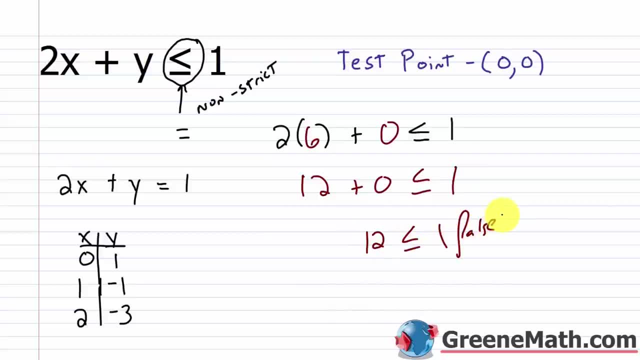 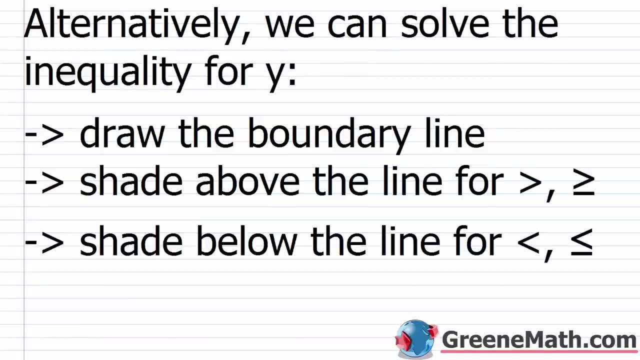 12 is not less than or equal to one, that's false. So that's kind of the first method you can use to do that. Now let me show you the fast way. So some books skip this altogether, and that should kind of make you a little mad, because 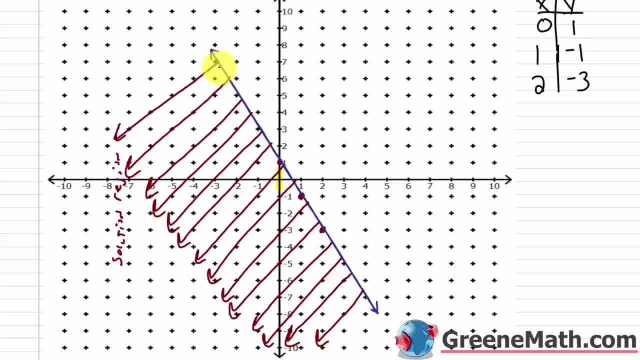 Okay, and over here, anything kind of above this line is the non-solution, non-solution region, and just try it out for yourself. 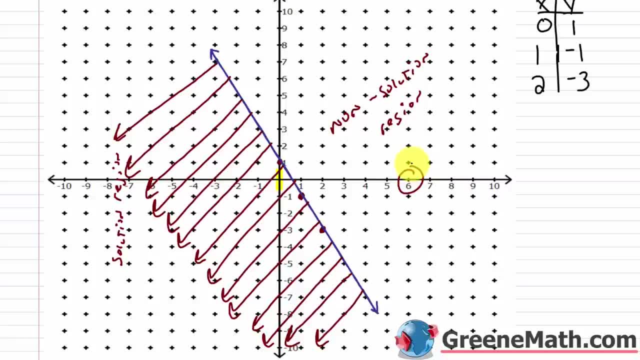 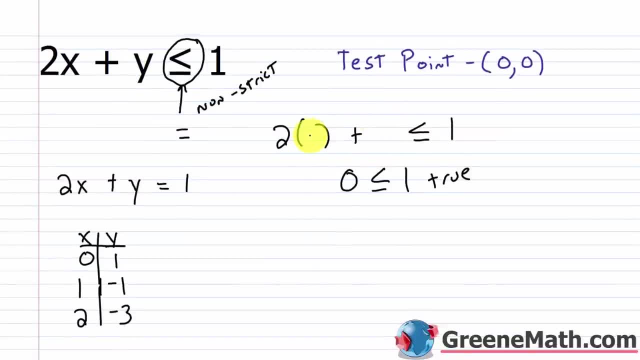 Pick some points over here. Pick 6,0, for example. That is in the non-solution region, so it shouldn't work. If I plug it in, I should get a false statement, so if I plug in a 6 for x and a 0 for y, I should get a false statement. 2 times 6 is 12. 12 plus 0 is not going to be less than or equal. 12 is not less than or equal to 1. That's false. 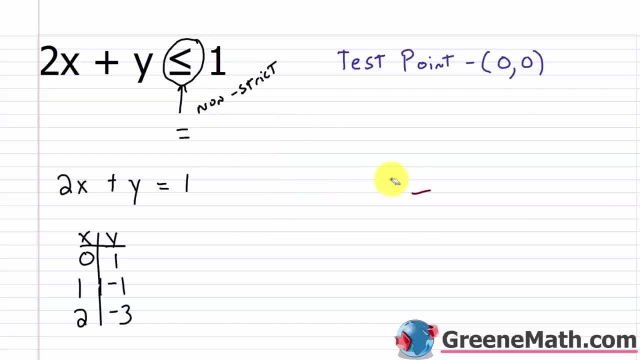 So that's kind of the first method you can use to do that. Now, let me show you the fast way. 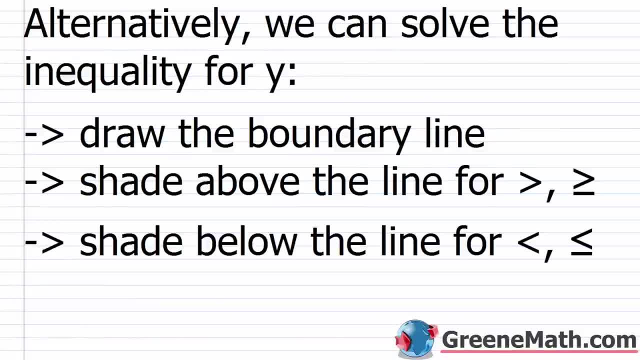 So some books skip this altogether, and that should kind of make you a little mad because this is way, way, way faster. 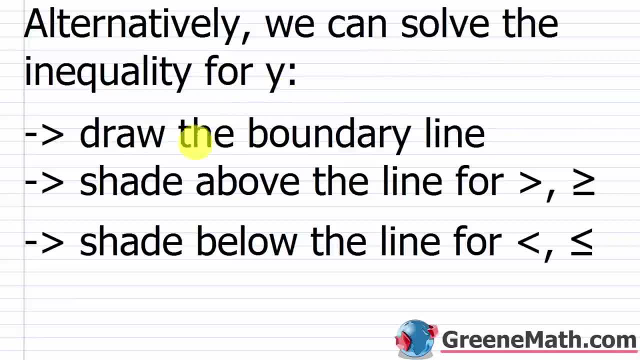 So alternatively, we can solve the inequality for y, draw the boundary line, same way, just replace the inequality symbol with an equal symbol, and then you shade above the line for greater than or greater than or equal to. You shade below the line for greater than or equal to. You shade below the line for less than or less than or equal to. 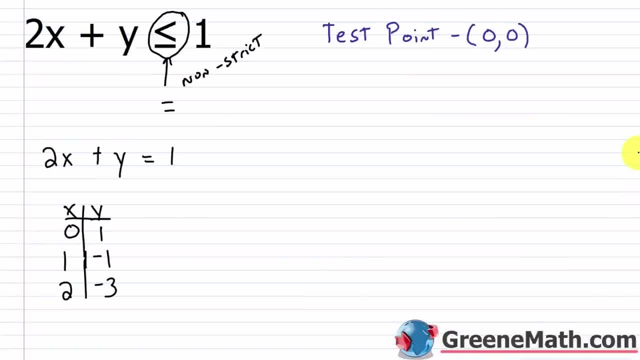 So in the previous example, I could have started out, I didn't need to get any ordered pairs, I could have just solved this guy for y. 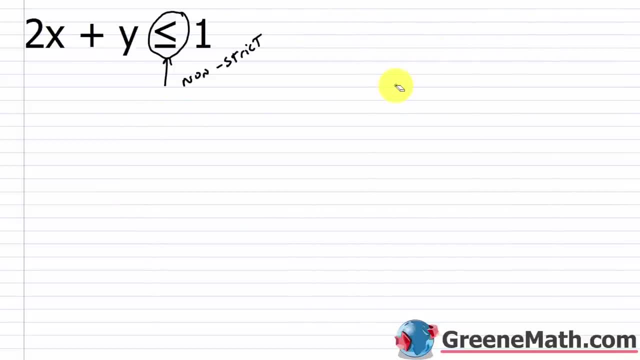 Forget about this test point, don't need that anymore. So solve it for y. 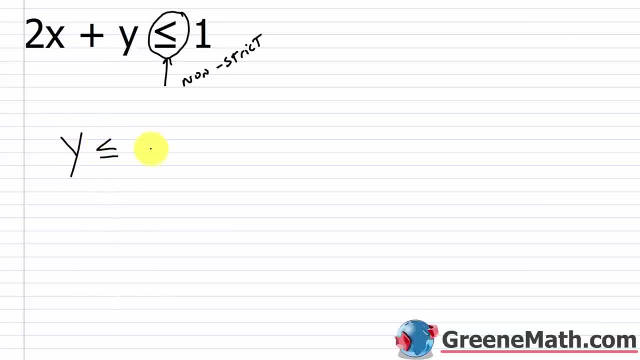 We have y is less than or equal to negative 2x plus 1. Now for the boundary line, I would replace this with equals, so I'd have y equals negative 2x plus 1. 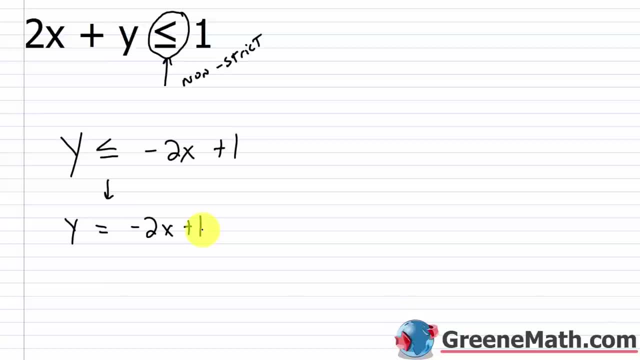 I know this is in slope-intercept form, so it's super easy to grasp. The y-intercept occurs at 0,1. 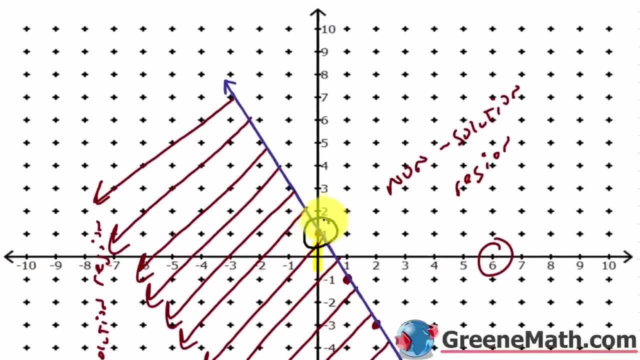 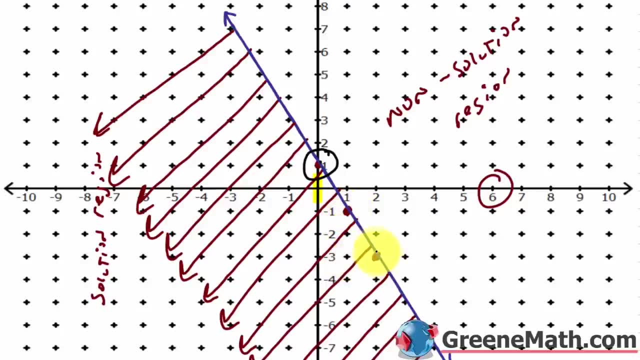 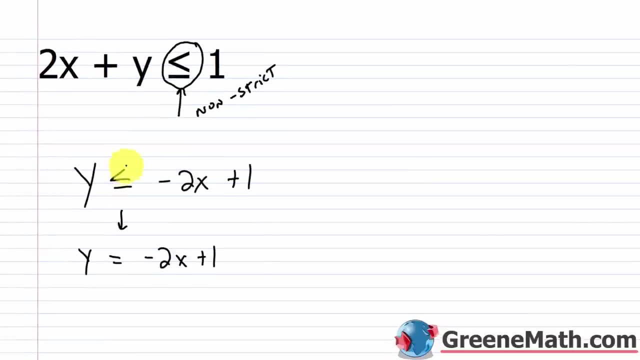 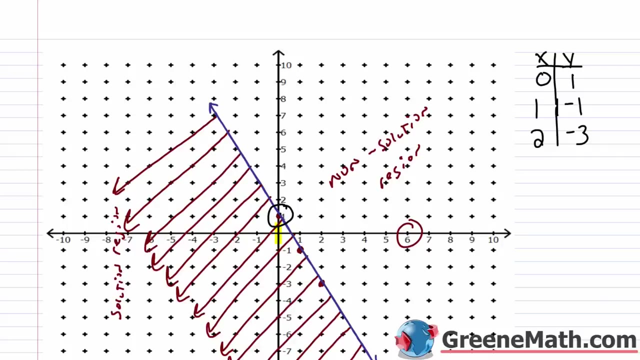 The slope is negative 2. So you can see I already have that point here, 0,1, and my slope is negative 2. So I go down 1,2 over 1, down 1,2 over 1. So I would graph the same line, so I'd come about that a little bit quicker. Now the next thing is the fact that it's less than or equal to. So if it's a less than, whether it's a less than or equal to or strictly a less than, you shade below the line, and that's what we did here. So we would just shade below the line, okay? Below the line. 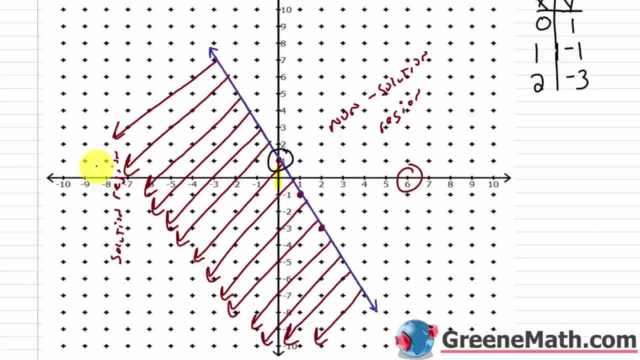 And once you get into a habit of doing it this way, it's much, much, much quicker. You don't need to worry about getting a test point and all this other stuff and going through and getting ordered pairs. 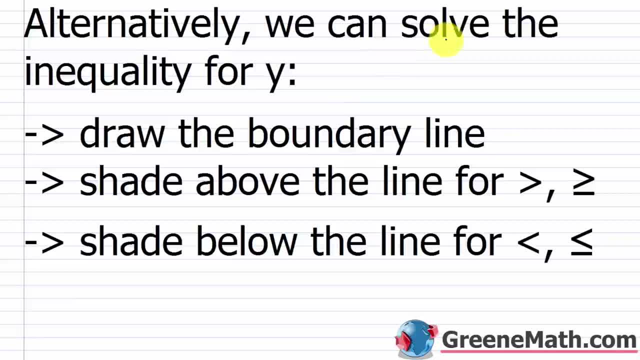 this is way, way, way faster. So, alternatively, we can solve the inequality for y, draw the boundary line same way, just replace the inequality symbol with an equal symbol And then you shade above the line for greater than, or greater than or equal to, you shade. 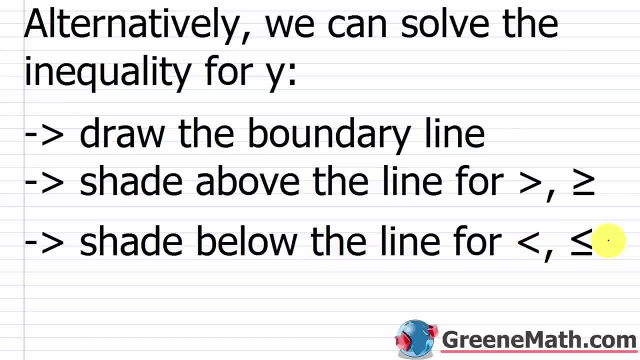 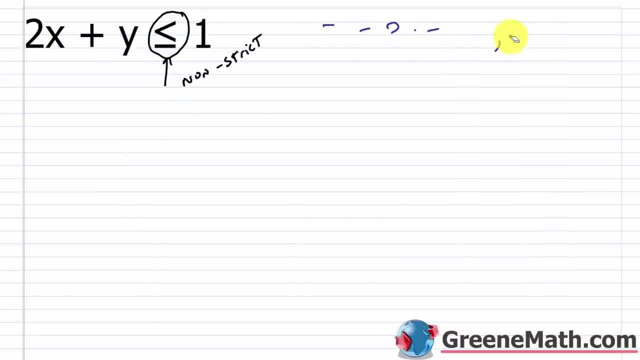 below the line for less than or less than or equal to. So in the previous example I could have started out. I didn't need to get any ordered pairs. I could have just solved this guy for y. Forget about this test point. don't need that anymore. 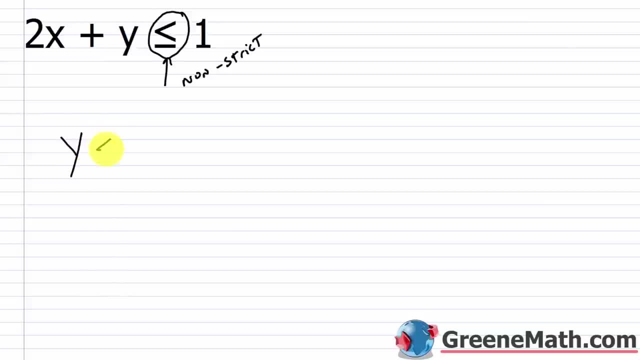 So solve it for y. We have: y is less than or equal to negative two x plus one. Now for the boundary line. I would replace this with equals, so I'd have y equals negative two x plus one. I know this is in slope intercept form so it's super easy to graph it. 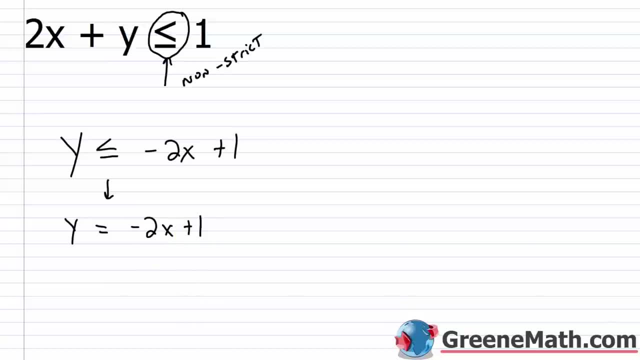 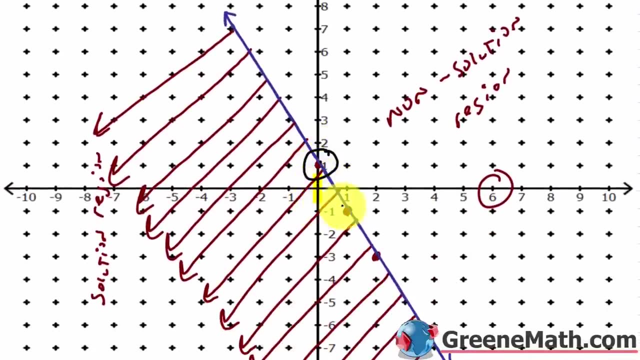 The y intercept occurs at zero comma one. The slope is negative two. So you can see I already have that point here: zero comma one and my slope is negative two. so I go down one two over one, down one two over one. 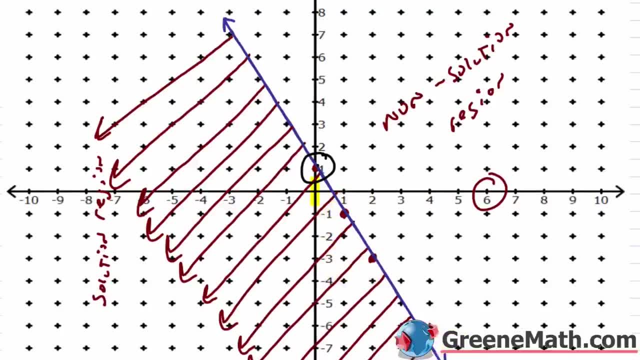 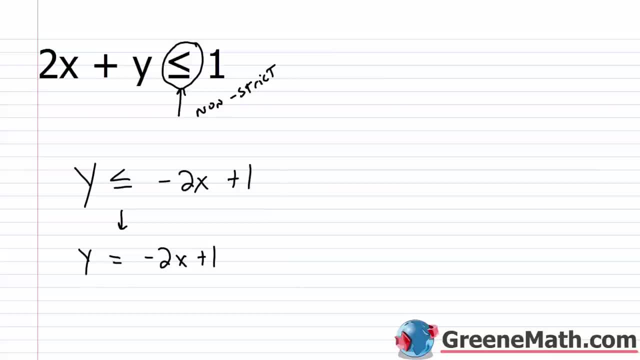 So I would graph the same line, so I'd come about that a little bit quicker. Now, the next thing is the fact that it's less than or equal to. so if it's a less than equal to, or strictly a less than, you shade below the line, and that's what we did here. 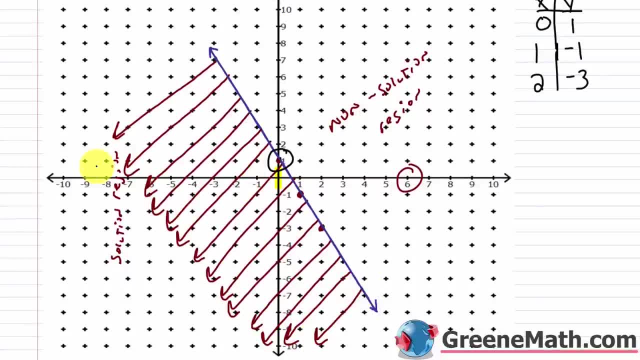 So we would just shade below the line. okay, below the line. and once you get into a habit of doing it this way, it's much, much, much quicker. You don't need to worry about getting a test point and all this other stuff and going through. 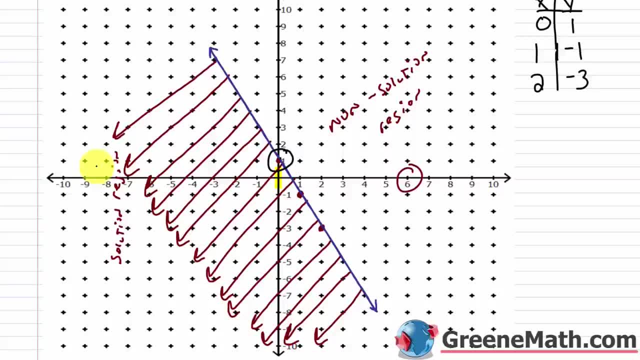 and getting ordered pairs. It's way quicker. So you're basically putting it into slope intercept form to graph it. Once you've done that, you look at the inequality that you're dealing with. if it's a less than, or it's a less than or equal to, it's below the line that you're going to shade. 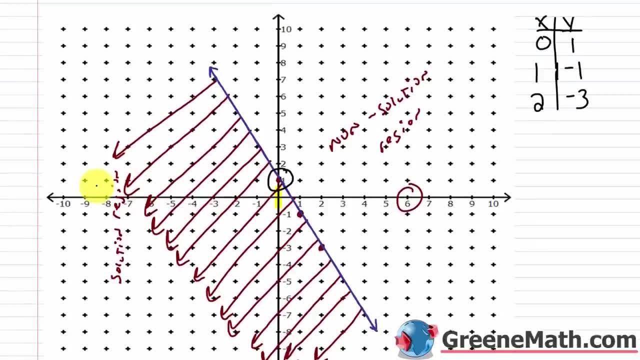 If it's a greater than, or a greater than or equal to, you just shade above the line. So for the next one, we look at seven x minus four. y is greater than negative eight. So we're going to do this the quick way. 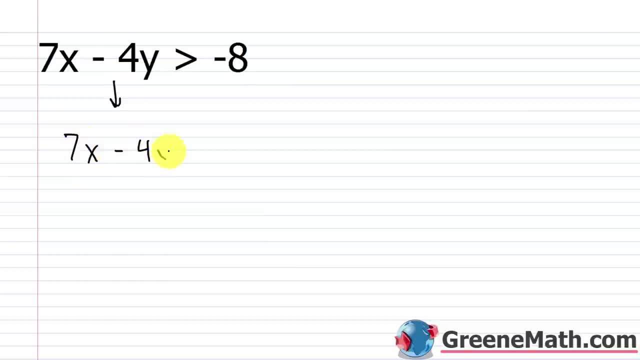 Let's just rewrite this real fast. We have seven x minus four. y is greater than negative eight. Solve it for y. So I'd subtract seven x from both sides of the inequality. I'd get negative four. y is greater than negative seven x minus eight. 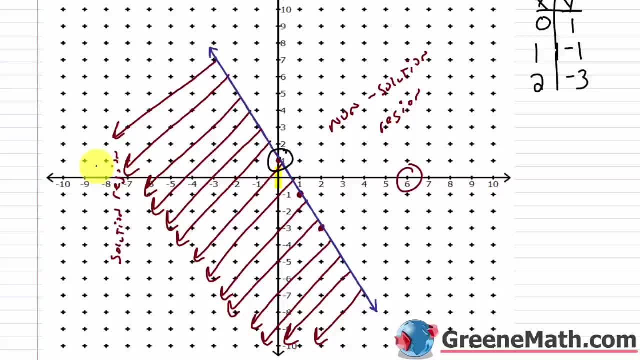 So you're basically putting it into slope-intercept form to graph it. Once you've done that, you look at the inequality that you're dealing with. If it's a less than or it's a less than or equal to, it's below the line that you're going to shade. If it's a greater than or a greater than or equal to, you just shade above the line. 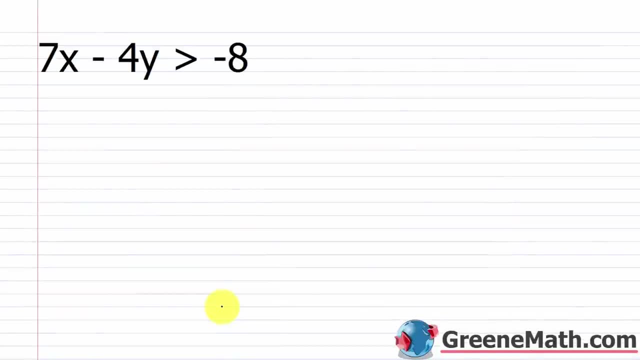 So for the next one, we look at 7x minus 4y is greater than negative 8. So we're going to do this the quick way. Let's just rewrite this real fast. 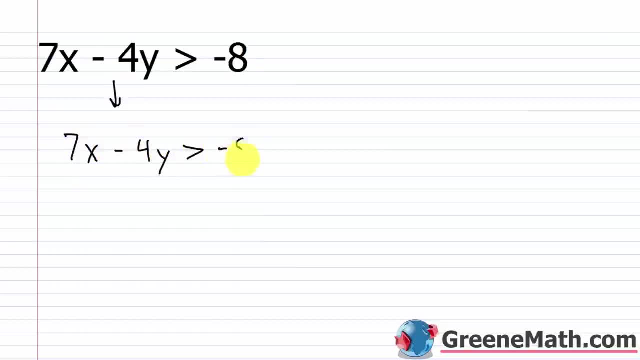 We have 7x minus 4y is greater than negative 8. Solve it for y. So I'd subtract 7x from both sides of the inequality. I'd get negative 4y is greater than negative 7x minus 8. Then I would divide both sides of the inequality by negative 4. But remember, if I divide by a negative, I've got to flip the inequality. 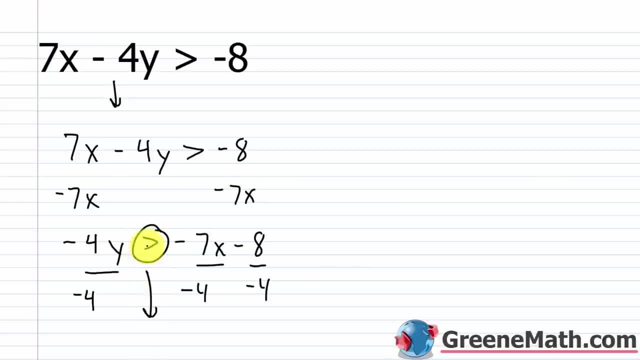 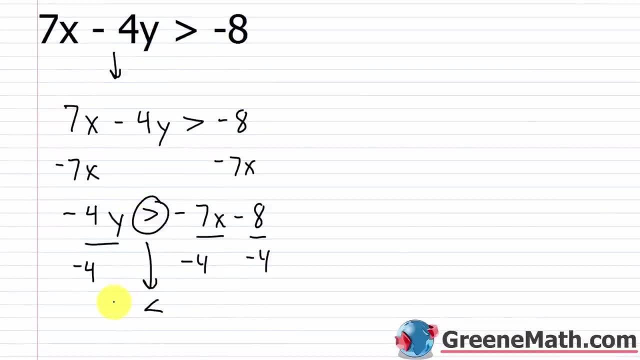 So instead of this being a greater than inequality, I'm going to have a less than. So that symbol there is going to flip from greater than to less than. So this is y is less than negative 7 divided by negative 4 is 7 fourths. Then times x. 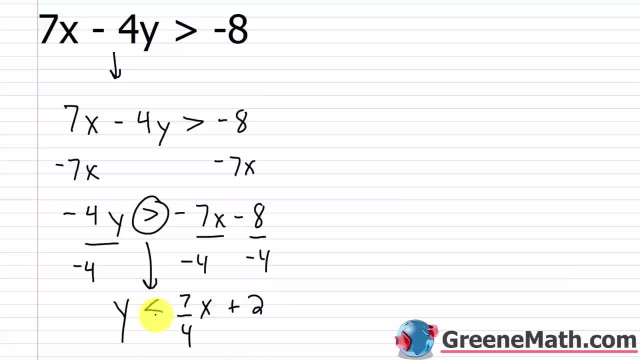 Negative 8 divided by negative 4 is plus 2. So if I replace this less than with an equals, I'd have y equals 7 fourths x plus 2. 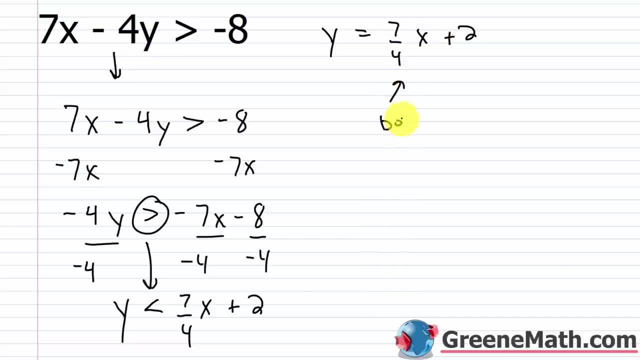 So that's y. Negative 7 divided by negative 4 is plus 2. So this is my boundary line. 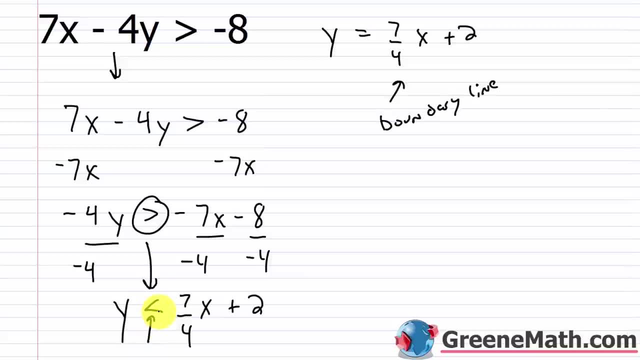 And you'll notice that this inequality is a strictly less than. 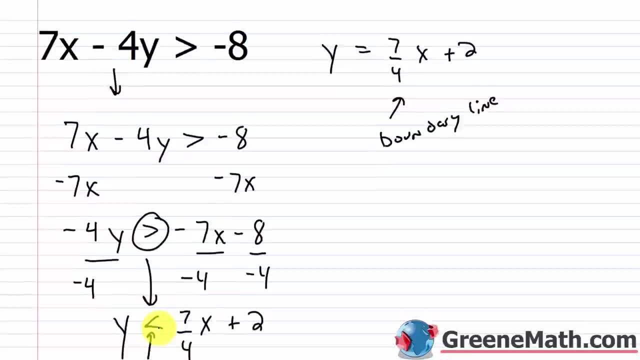 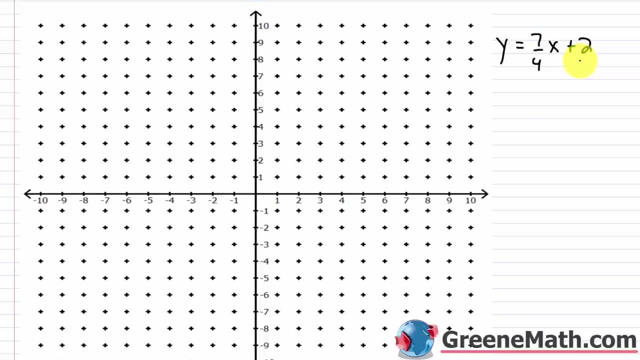 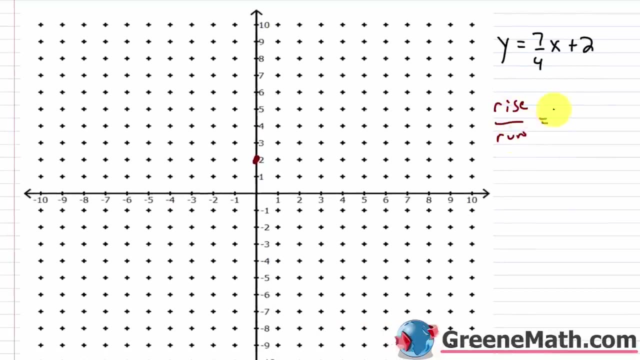 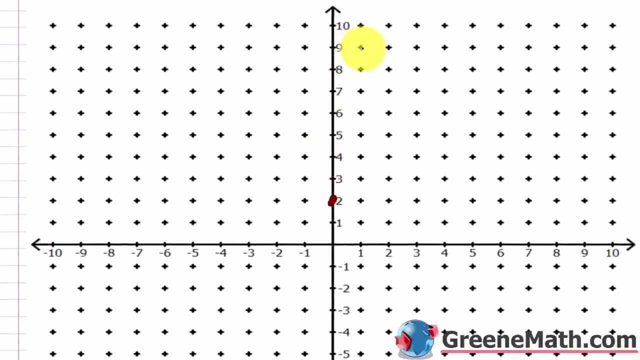 So I want to make sure that I have a broken or dashed line. So y equals 7 fourths x plus 2. That's what I'm going to graph. So my y intercept occurs at 0 comma 2. It's right there. And my rise over run is 7. It's 7 over 4. So I go up 7, 1, 2, 3, 4, 5, 6, 7, to the right 4, 1, 2, 3, 4. 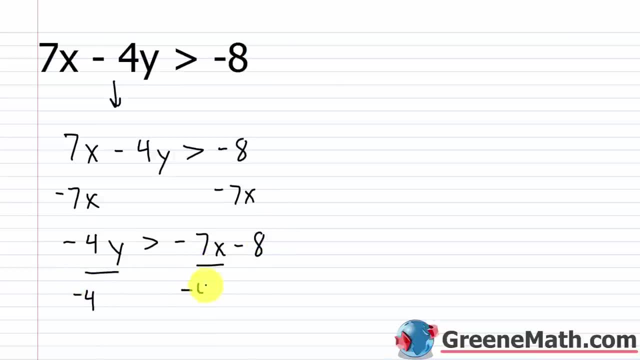 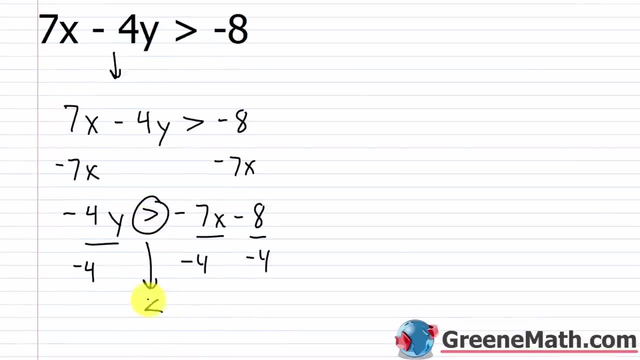 Then I would divide both sides of the inequality by negative four. But remember, if I divide by a negative, I've got to flip the inequality. So instead of this being a greater than inequality, I'm going to have a less than. So that symbol there is going to flip from greater than to less than. 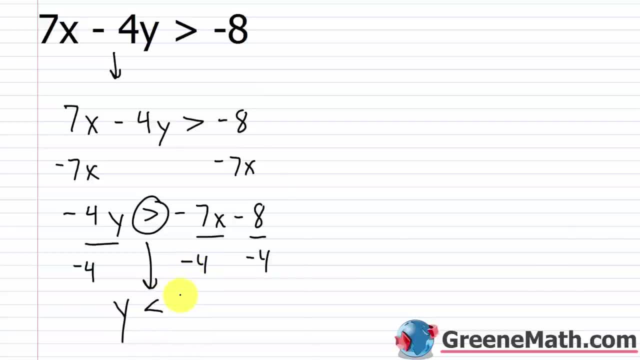 So this is: y is less than negative seven divided by negative four is seven fourths. then times x negative eight divided by negative four is plus two. So if I replace this less than with an equal, I'd have y equals seven fourths x plus two. 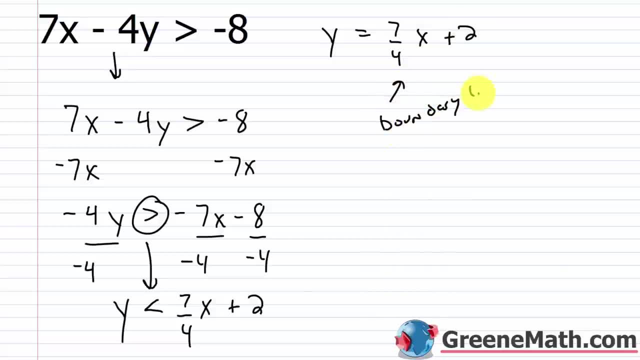 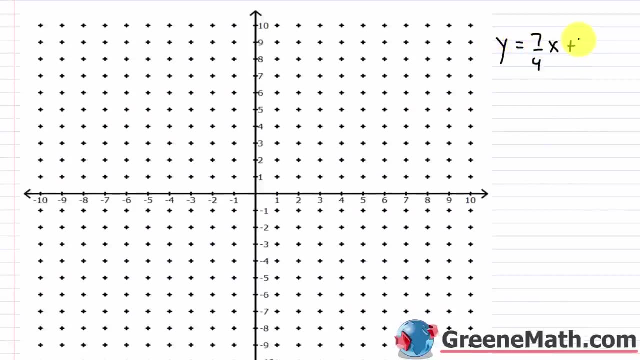 So this is my boundary line, And you'll notice that this inequality is a strictly less than So I want to make sure that I have a broken or dashed line. So y equals seven fourths x plus two. That's what I'm going to graph. 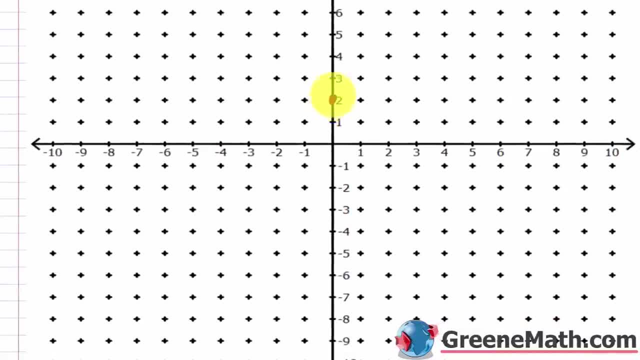 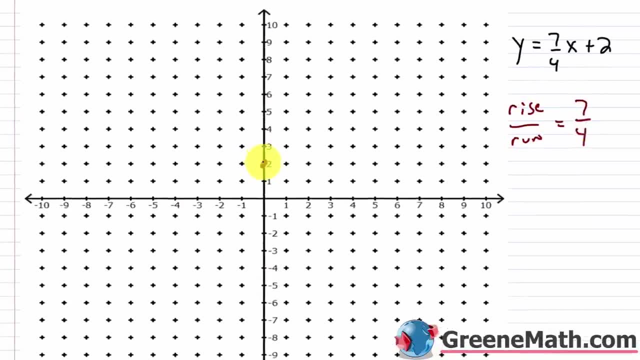 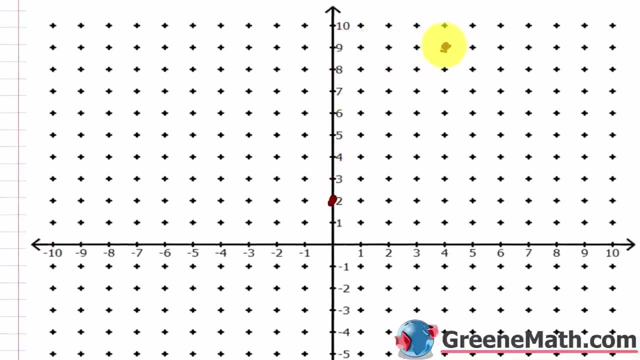 So my y intercept occurs at zero, comma two. it's right there. So I have me cause these, and these are based off of a quantum un energized equation. What you're going to do is see here Again, I got taller. My y's overrun is seven over four. 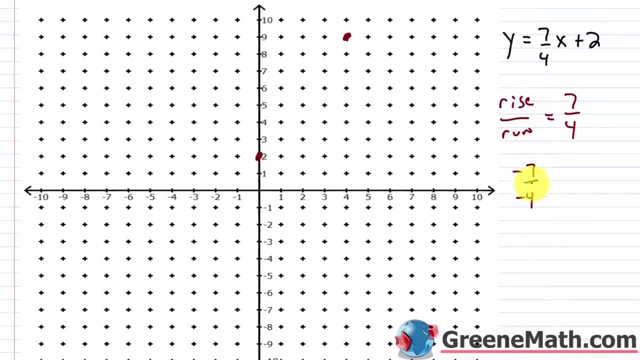 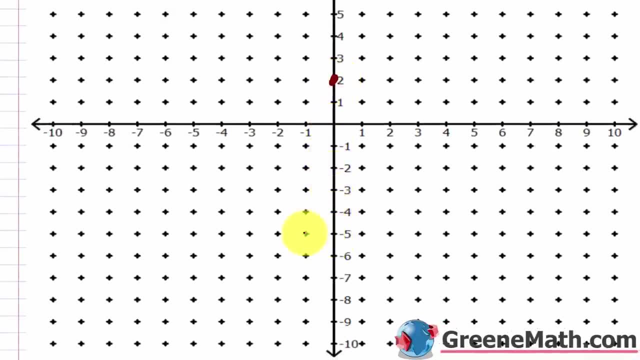 So I go up seven: one, two, three, four, five, six, seven to the right: four: one, two, three, four, and I can do that using negative seven over negative, four as well, negative over negatives, positive, So I can fall seven. 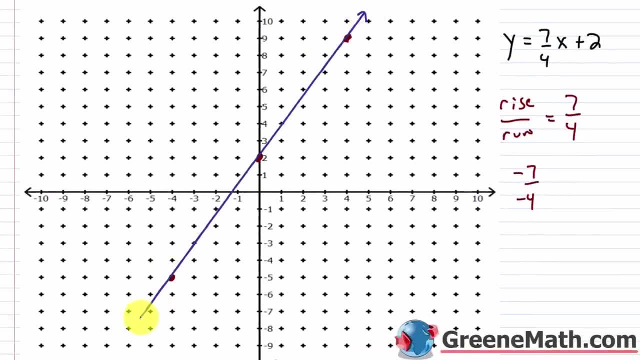 One, two, three, four, five, six, seven. So I start out by just drawing a solid line and then I take my eraser and I just kind of break it up. So just break it up good enough to where your teacher or whoever's grading your work can. 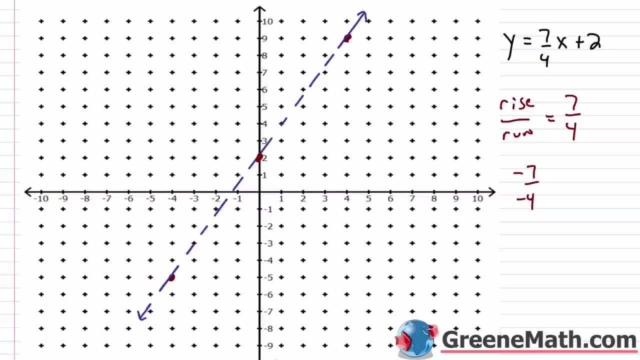 see that that line is broken or dashed. Okay, so this is an example of a dashed line. Let me kind of break that up a little bit too. So that tells me that an ordered pair that exists on that line is not going to be involved. 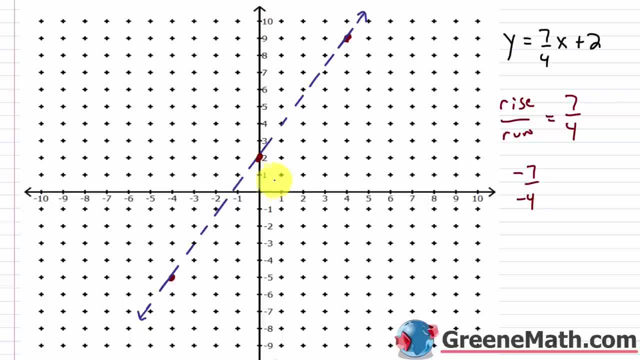 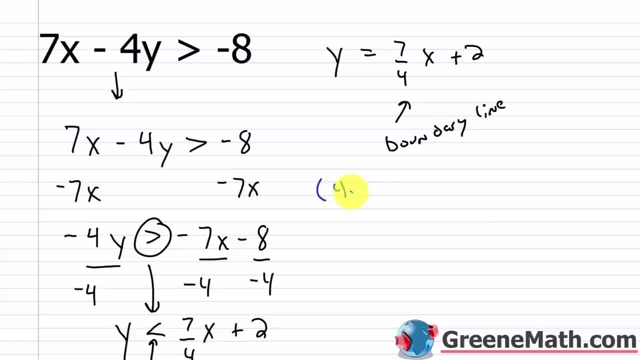 in the solution. So, for example, the point four comma nine will not be a solution and we'll test that in a minute. Let me just write that we're going to test four comma nine. Before we do that, remember this is a strictly less than. 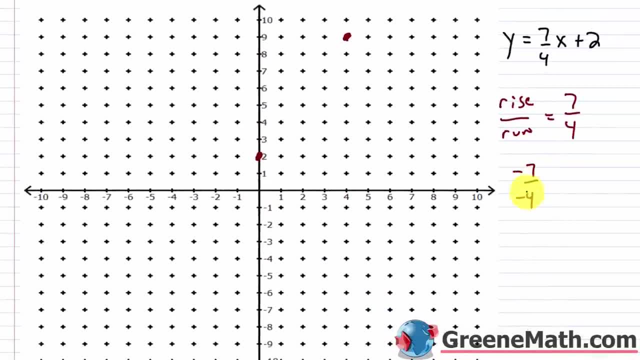 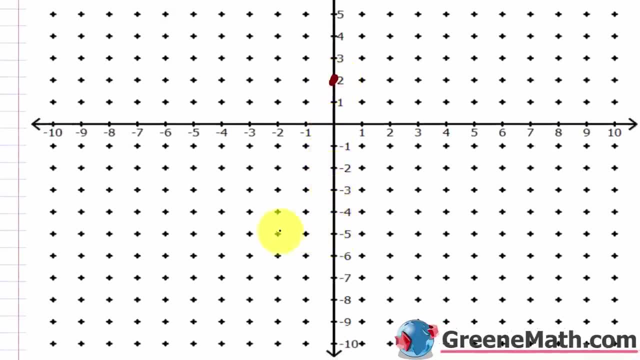 And I can do that using negative 7 over negative 4 as well, negative over negative is positive. So I can fall 7, 1, 2, 3, 4, 5, 6, 7, and to the left 4, 1, 2, 3, 4. 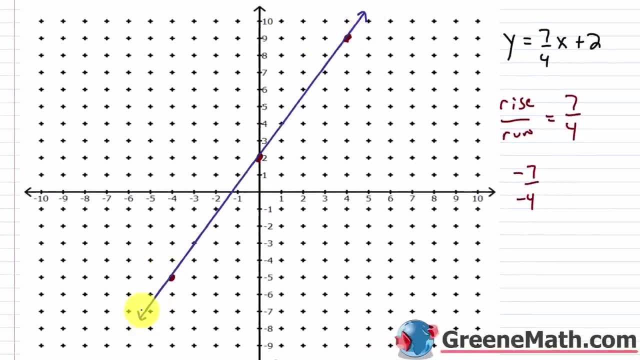 So I start out by just drawing a solid line. And then I take my eraser and I just kind of break it up. So just break it up good enough to where your teacher or whoever is grading your work can see that that line is broken or dashed. Okay. So this is an example of a dashed line. Let me kind of break that up a little bit too. 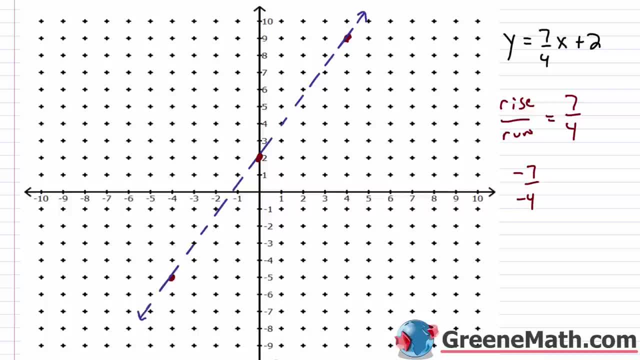 So that tells me that an ordered pair that exists on that line is not going to be involved in the solution. So for example, the point 4 comma 9. Okay. 4 comma 9 will not be a solution. And we'll test that in a minute. 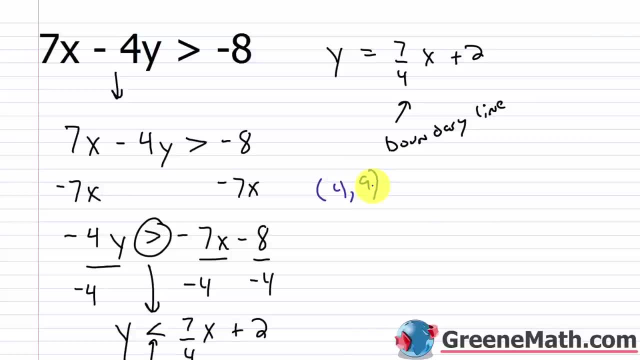 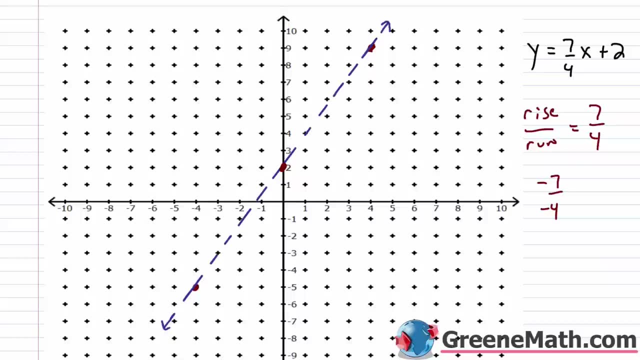 Let me just write that we're going to test 4 comma 9. Before we do that, remember this is a strictly less than. So that tells me I want to shade below the line. 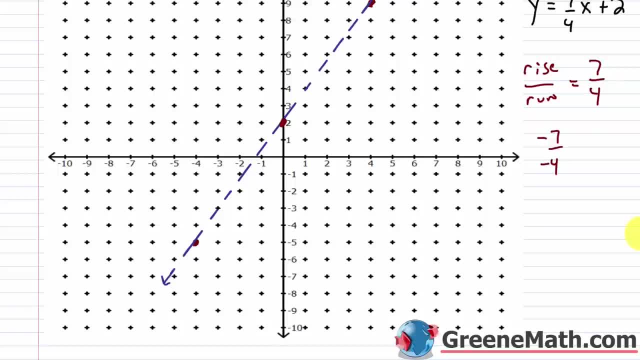 So when I shade this, I'm going to shade below the line, all this. 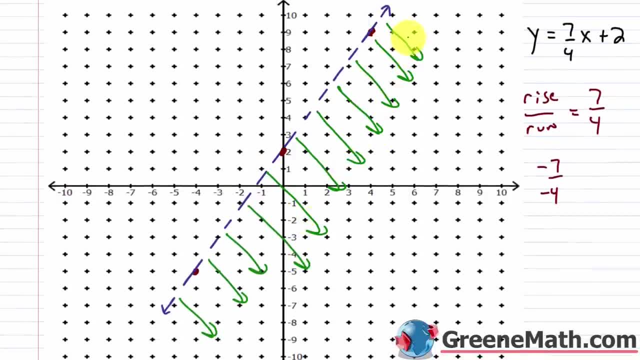 That's all you need to do is give your teacher a representation of where the solution region is going to be. Just shade all of this. Okay. 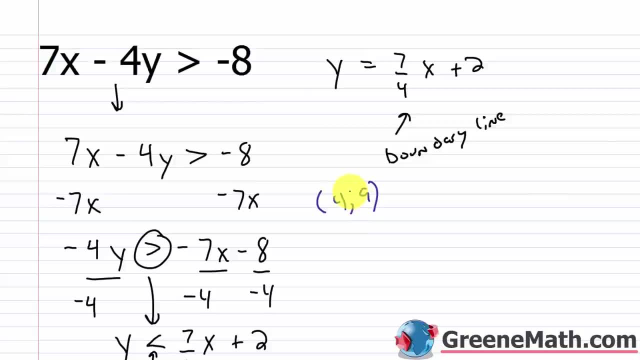 So let's test a few things. So let's test 4 comma 9 in the original inequality. I'm going to erase all of this. I don't need it. 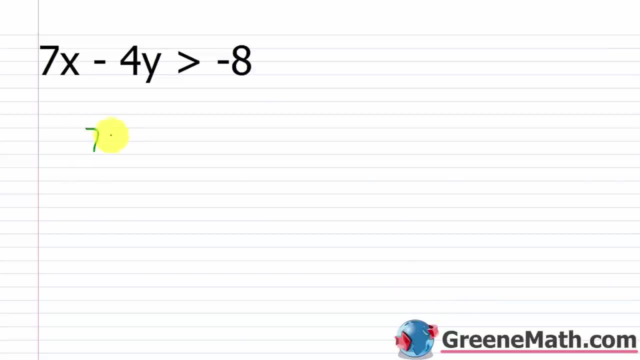 We'll show you this doesn't work. So it lies on that boundary line. So 7 times 4 minus 4 times 9 is greater than negative 8. 7 times 4 is 28 minus 4 times 9 is 36. This is greater than negative 8. So 28 minus 36 is negative 8. That's not greater than negative 8. But. 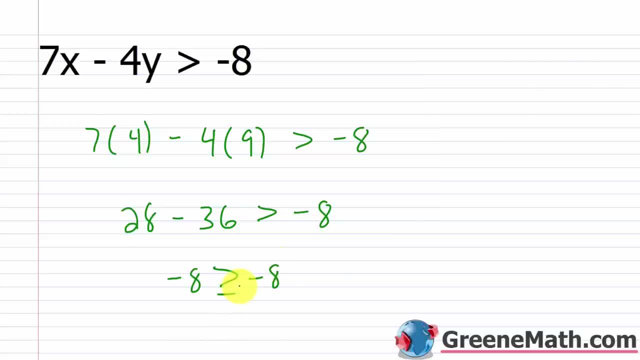 Remember, if I had a greater than or equal to here, this would end up being true. 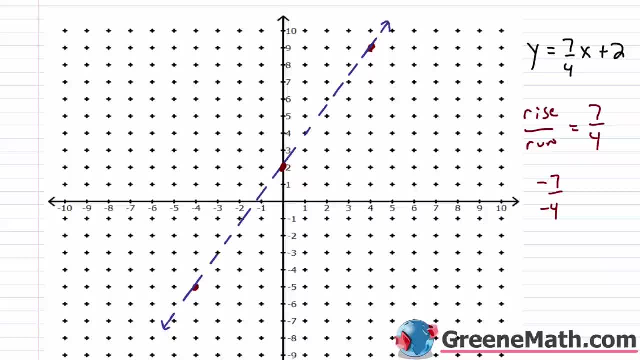 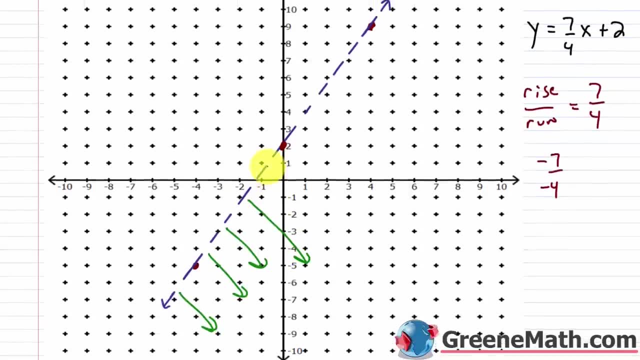 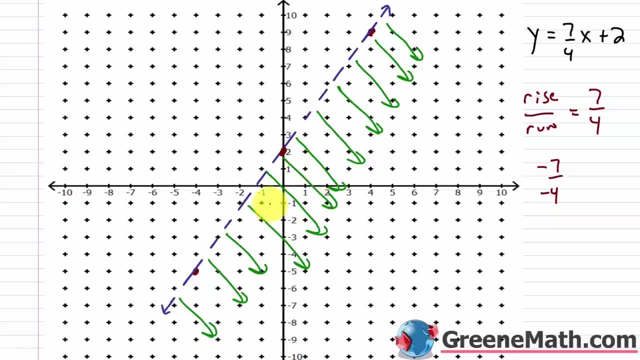 So that tells me I want to shade below the line. So when I shade this, I'm going to shade below the line. All this, That's. all you need to do is give your teacher a reference. This is a representation of where the solution region is going to be. 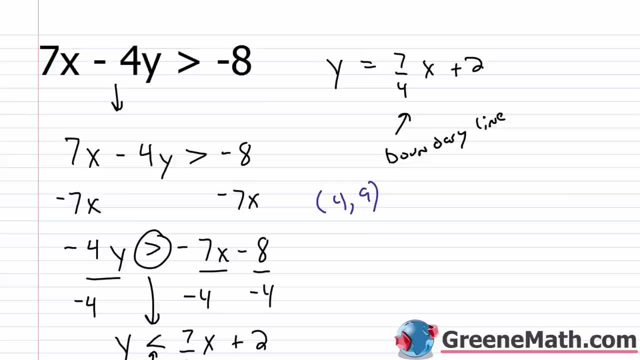 Just shade all of this, Okay, so let's test a few things. So let's test four comma nine in the original inequality. I'm going to erase all of this. I don't need it. We'll show you. this doesn't work. 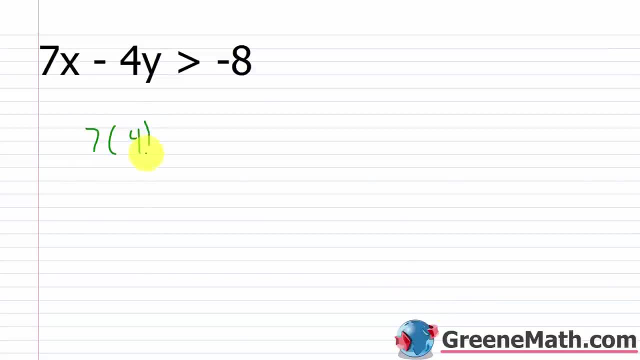 So it lies on that boundary line. So seven times four minus four times nine is greater than negative eight. Seven times four is 28 minus four times nine is 36.. This is greater than negative eight, So 28 minus 36.. Six is negative eight. 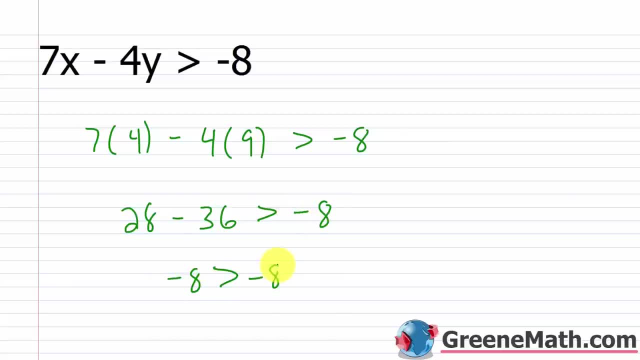 That's not greater than negative eight. But remember, if I had a greater than or equal to here, this would end up being true. So that's the difference between having a strict inequality and a non-strict inequality. Again, if you have a strict inequality like we have here, we do not allow, okay. 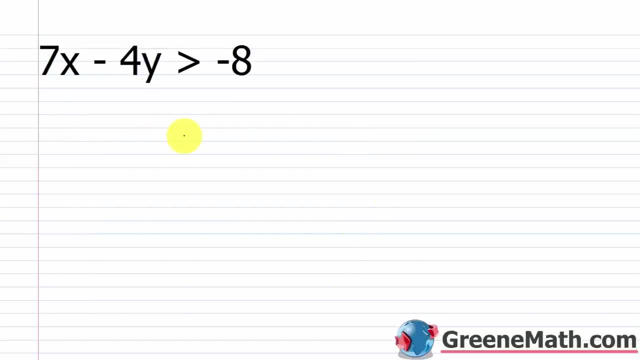 we do not allow for anything on that boundary line to be part of the solution for that reason that I just showed you. So we break it up to say, hey, nothing on this line. It works With a non-strict inequality. the things on the line do work as solutions. 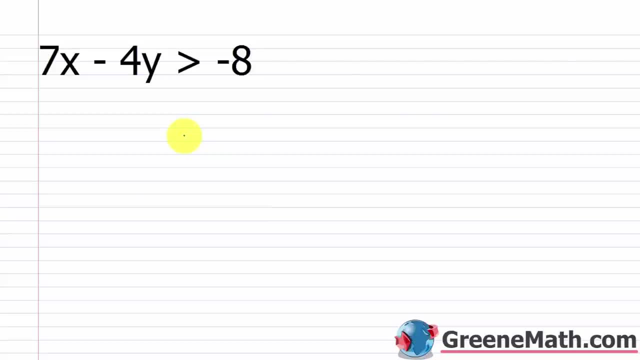 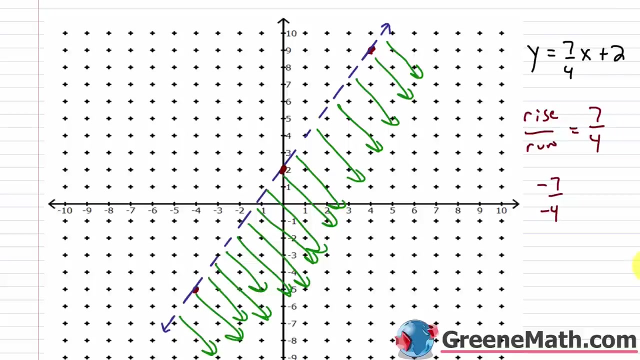 So you got to draw a solid line for your boundary line when you have a non-strict inequality and a broken or dashed line for a strict inequality. Now one more thing I want to just bring your attention to. If we use the test point here, we could still see that we have the right answer. 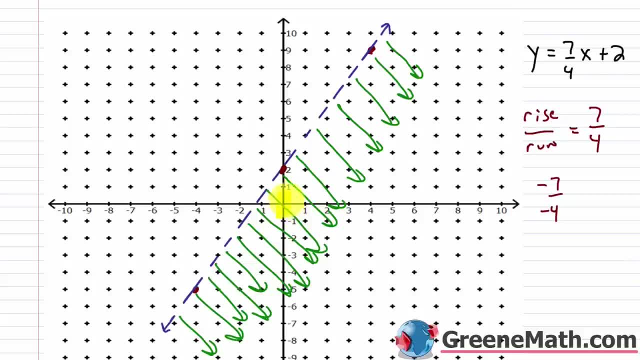 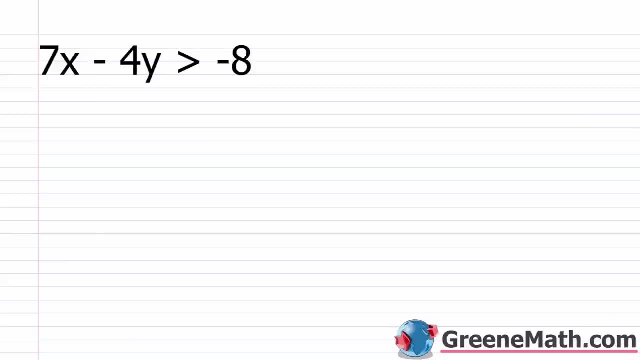 You could pick something in the solution region. Again, zero comma zero. the origin is very, very easy to use, So that's something that should work. So let's go back up and test it. Let's see if zero comma zero works as it should. 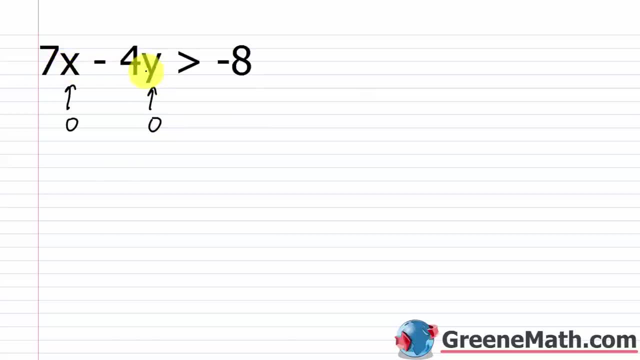 Plug in a zero here and here. Zero minus zero, which is zero, should be greater than negative eight. That is true, Okay, So zero comma zero should be in the solution region, and it is right because it does work. 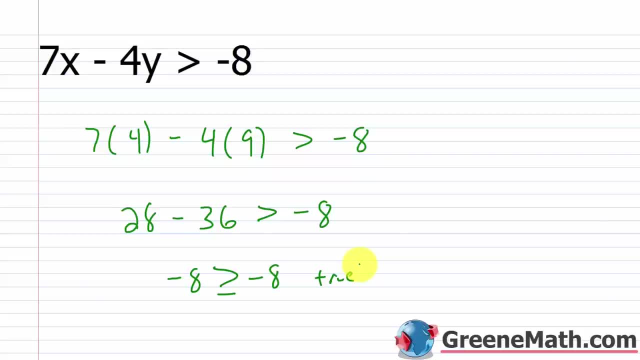 So that's the difference between having a strict inequality and a non-strict inequality. Again, if you have a strict inequality like we have here, we do not allow, okay, we do not allow for anything on that boundary line to be part of the solution for that reason that I just showed you. 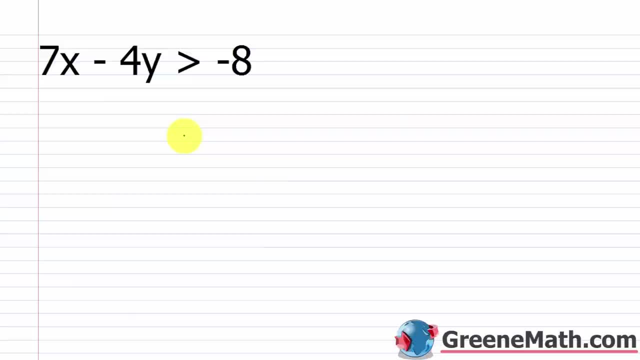 So we break it up to say, hey, nothing on this line works. With a non-strict inequality. The things on this line are not going to work. The things on the line do work as solutions. So you got to draw a solid line for your boundary line when you have a non-strict inequality and a broken or dashed line for a strict inequality. 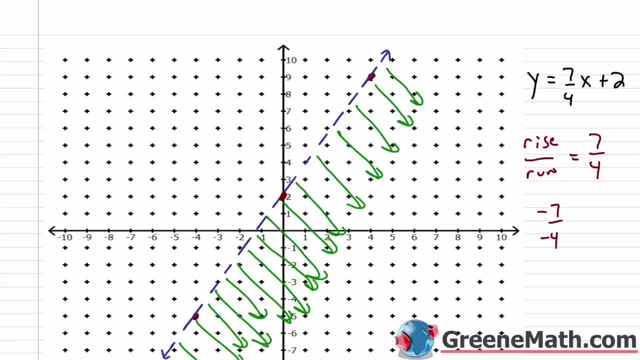 Now one more thing I want to just bring your attention to. If we use the test point here, we could still see that we have the right answer. 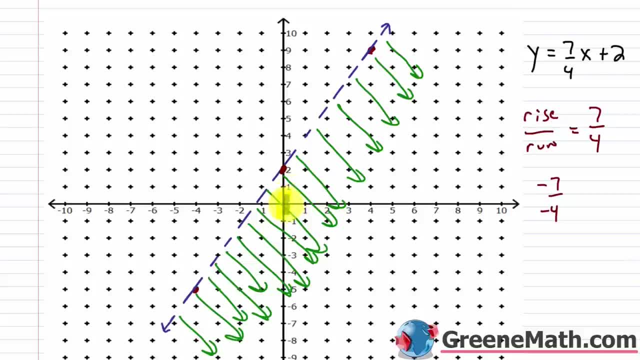 You could pick something in the solution region. Again, 0 comma 0, the origin is very, very easy to use. So that's something that should work. 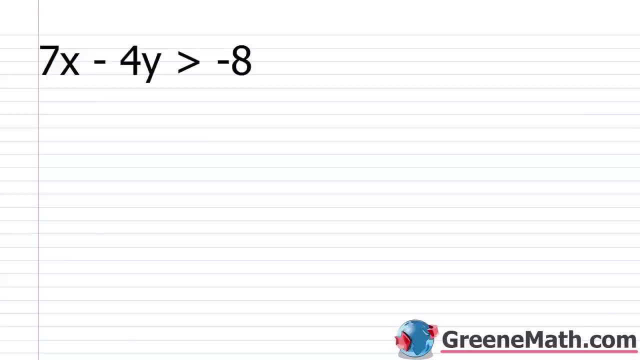 So let's go back up. And test it. Let's see if 0 comma 0 works as it should. Plug in a 0 here and here. 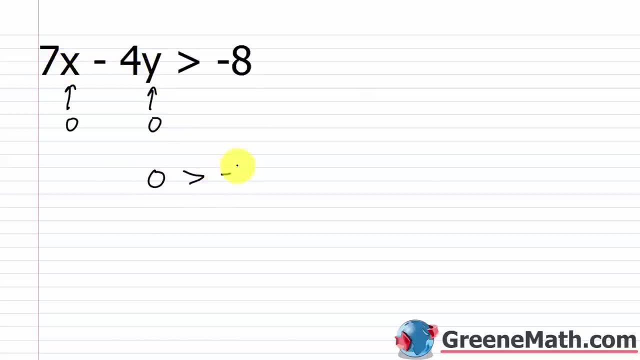 0 minus 0, which is 0, should be greater than negative 8. That is true. Okay. 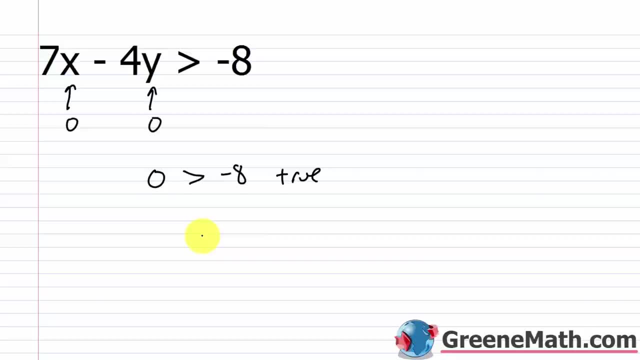 So 0 comma 0 should be in the solution region. And it is, right? Because it does work. 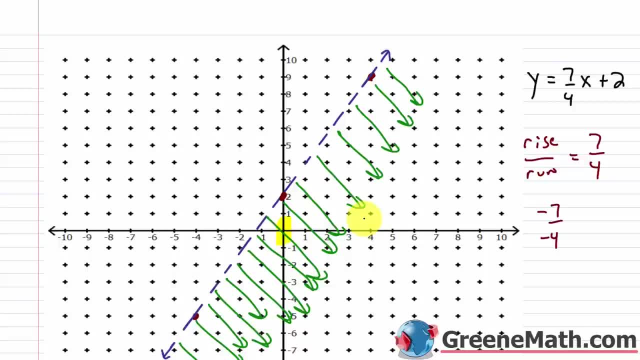 So you can kind of use that as a little check to show that you graphed the correct region. All right. Let's take a look at a few special case scenarios. 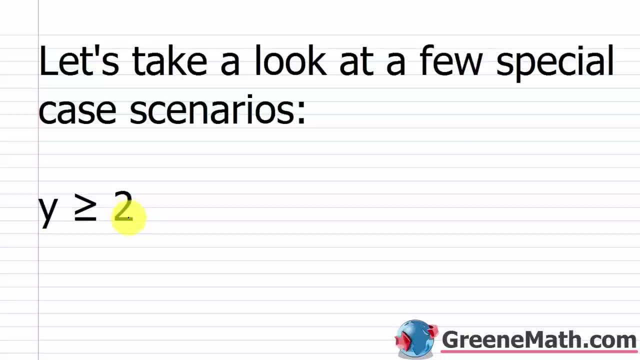 So something like y is greater than or equal to 2. Well. 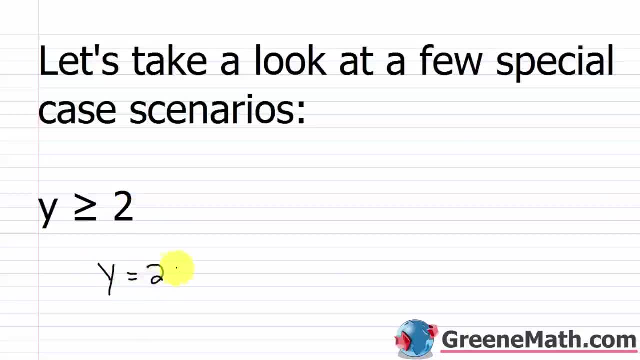 We saw that if we had something like y is equal to 2, this is a horizontal line, right? So we would find 2 on the y-axis, and we would draw a horizontal line. We're essentially going to do the same thing for something like this. So y is greater than or equal to 2. It's a non-strict inequality. So my boundary line will be a solid line. I'm going to find 2 on my y-axis. 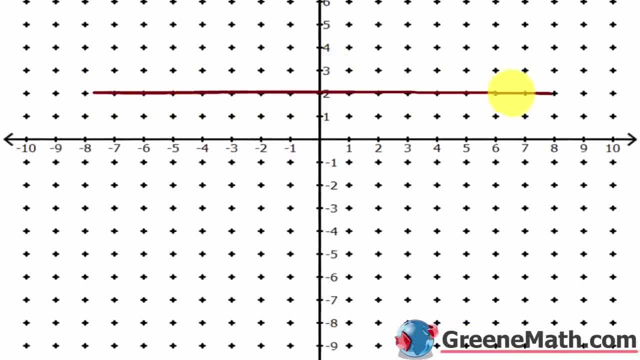 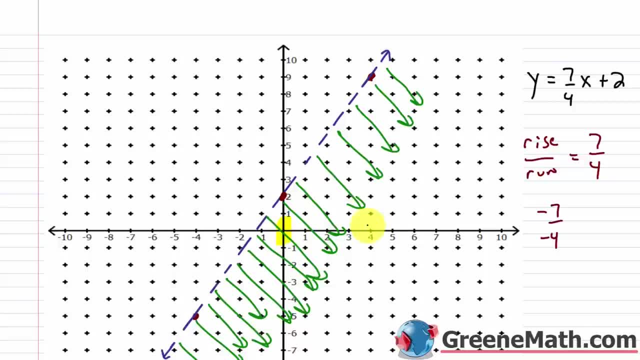 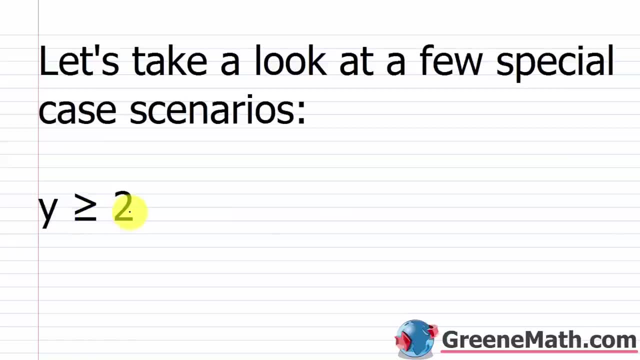 So you can kind of use that as a little check to show that you graphed the correct region. All right, let's take a look at a few special case scenarios. So something like y is greater than or equal to two. Well, we saw that if we had something like y is equal to two, this is a horizontal line, right? 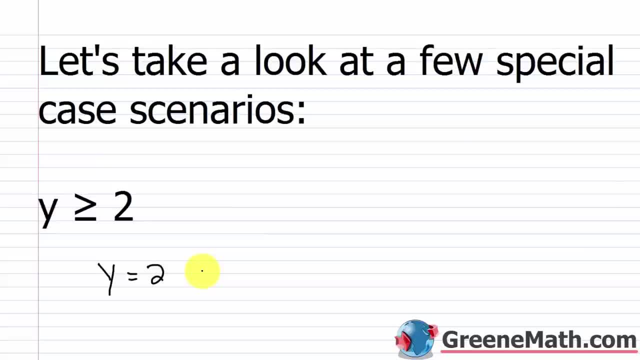 So we would find two on the y-axis and we would draw a horizontal line. We're essentially going to do the same thing for something like this. So y is greater than or equal to two. It's a non-strict inequality. So my boundary line will be a solid line. 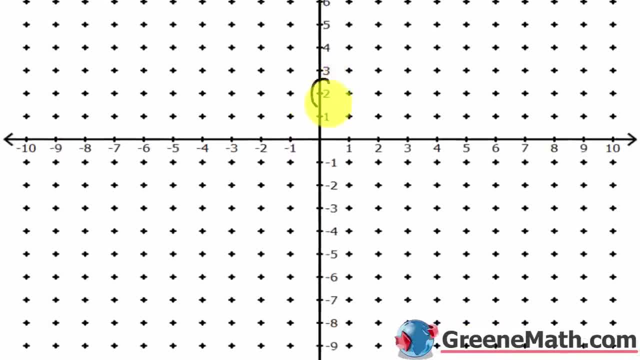 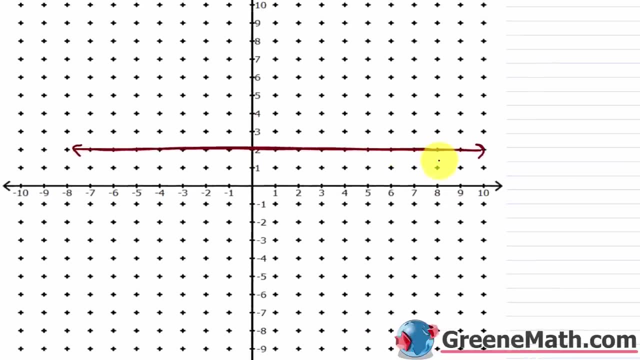 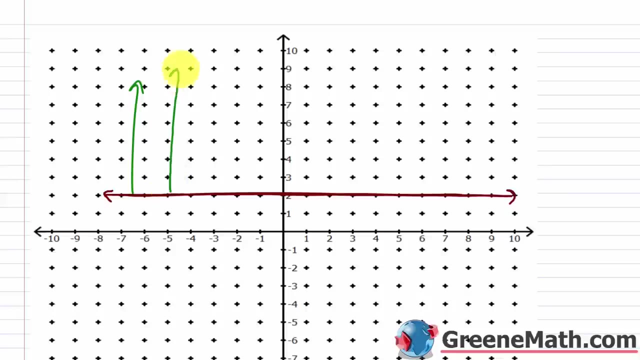 I'm going to find two on my y-axis, so that's right here. Okay, So this would be the line: y equals two. Again, that's our boundary line in this case. Now, because y was a greater than or equal to, I'm just going to shade above this line. 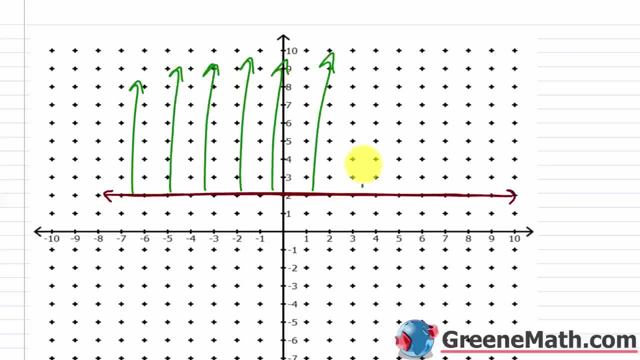 because y is anything that is greater than or equal to two. Again, no matter what the x value is, it's going to work because the y value that's given will be larger or equal to two. So if I pick something like I don't know, let's say an x value of five and a y value of ten. 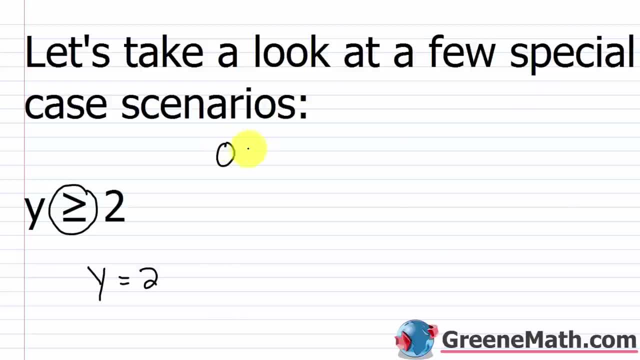 Well, again, I could represent this by saying: I have zero: x plus y is greater than or equal to two. So whatever I plug in for x just goes away. So I plug in the value for y, I plug in a ten: Ten is greater than or equal to two. 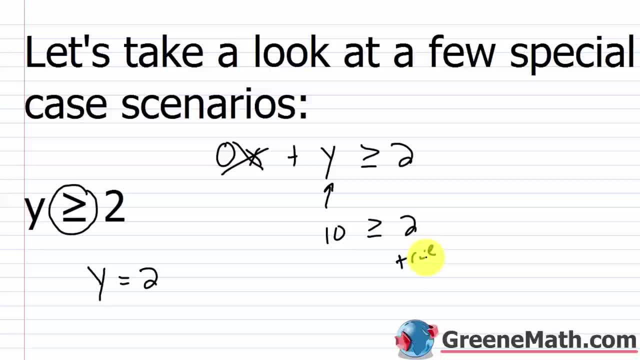 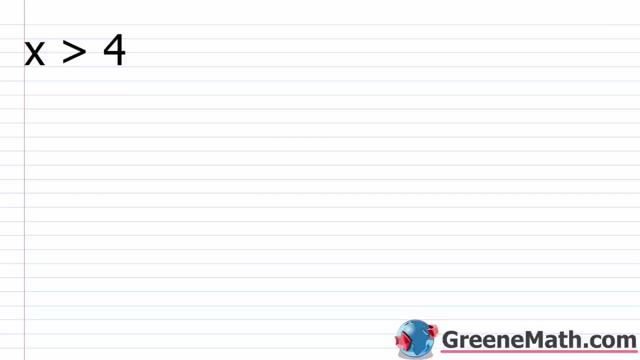 Yeah, ten is greater than two, so this is true. All right, so you can see how that's a very easy scenario to deal with. All right, so another easy one would be something like x is greater than four. So we saw that x equals four is a vertical line. 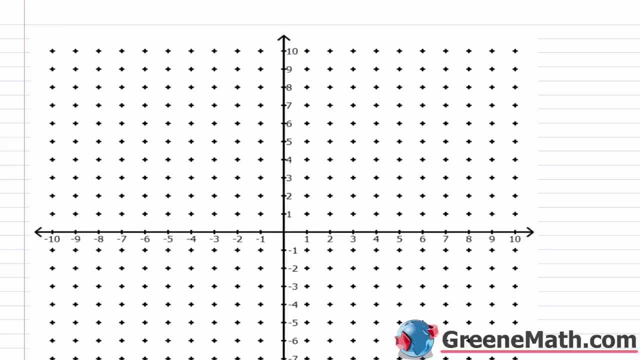 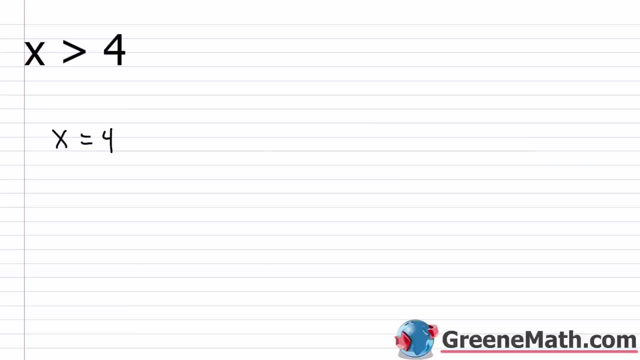 So I would find four on the x-axis- That's right here- And I would draw a vertical line. But here's the key, Because we have a strict inequality. this is strict. I can't include that line as part of the solution. 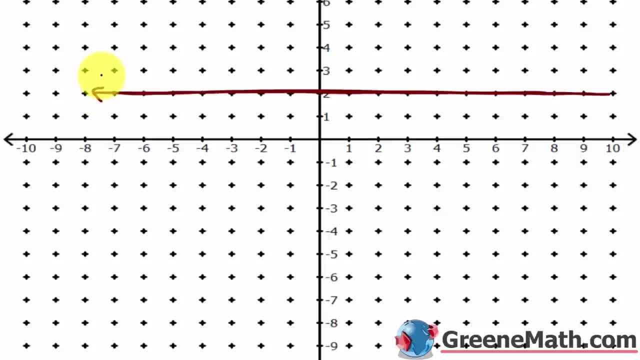 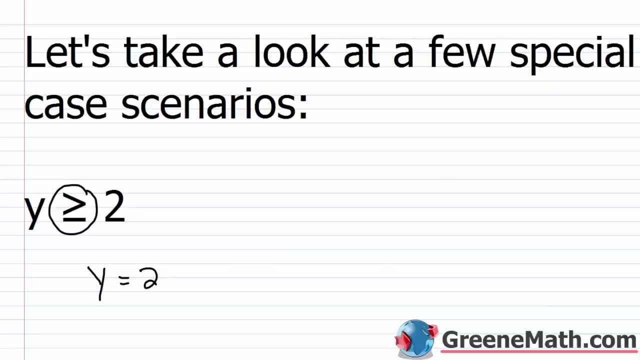 So this would be the line y equals 2. And again, that's our boundary line in this case. 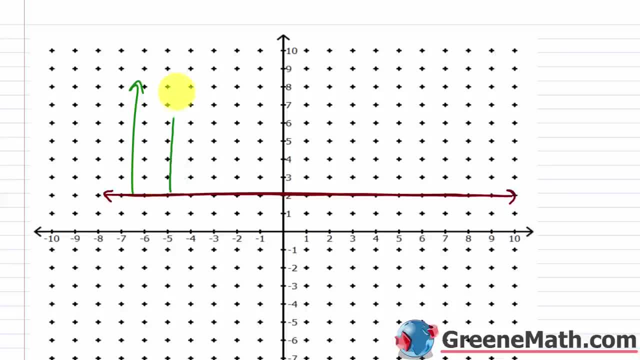 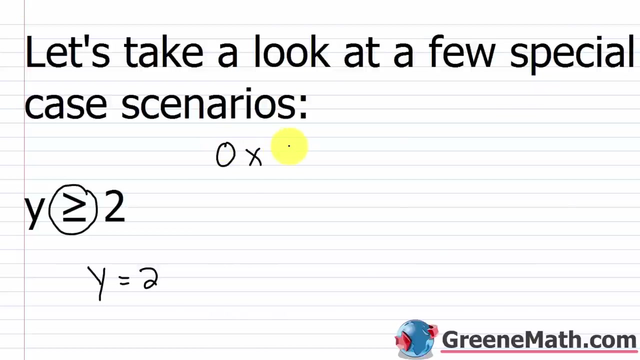 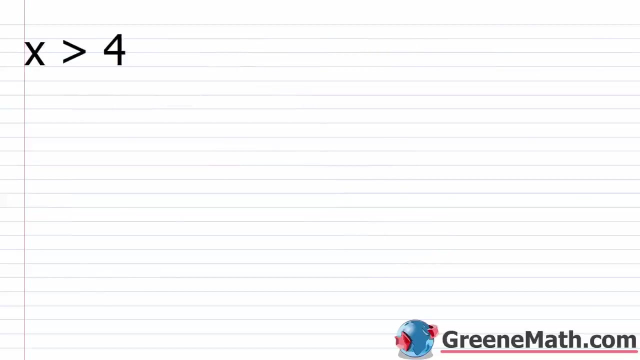 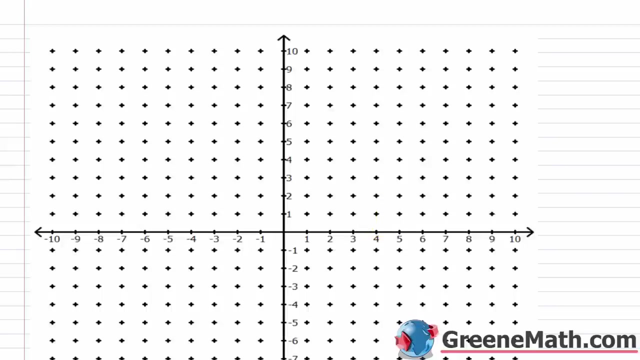 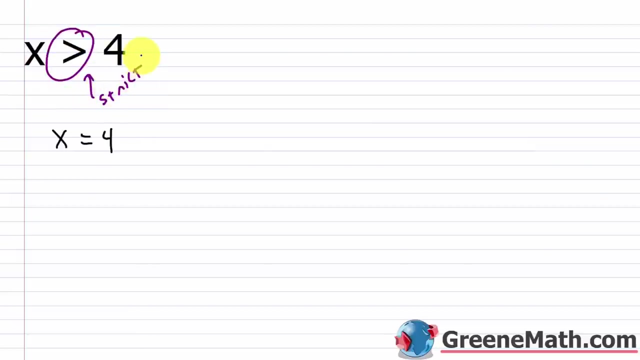 Now because y was a greater than or equal to, I'm just going to shade above this line. Because y is anything that is greater than or equal to 2. And again, no matter what the x value is, it's going to work because the y value that's given will be larger or equal to 2. So if I pick something like, I don't know, let's say an x value of 5 and a y value of 10. Well, again, I could represent this by saying I have 0x plus y is greater than or equal to 2. So whatever I plug in for x just goes away. So I plug in the value for y, I plug in a 10. 10 is greater than or equal to 2. Yeah, 10 is greater than 2, so this is true. All right, so you can see how that's a very easy scenario to deal with. All right, so another easy one would be something like x is greater than 4. So we saw that x equals 4 is a vertical line. So I would find 4 on the x-axis. That's right here. And I would draw a vertical line. But here's the key. Because we have a strict inequality, this is strict, I can't include that line as part of the equation. So I can't include that line as part of the equation. So I can't include that line as part of the solution. So I've got to kind of break it up or make it dashed. 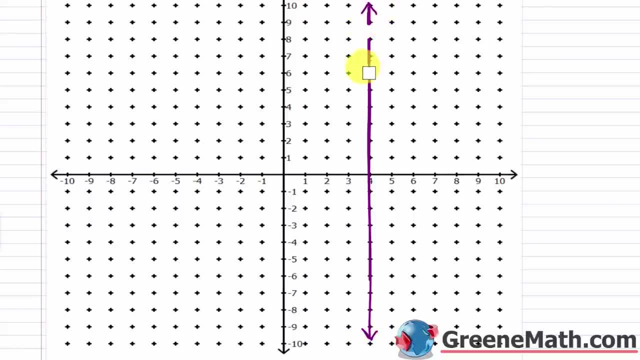 And now I'm going to take my eraser, just take chunks out of it. 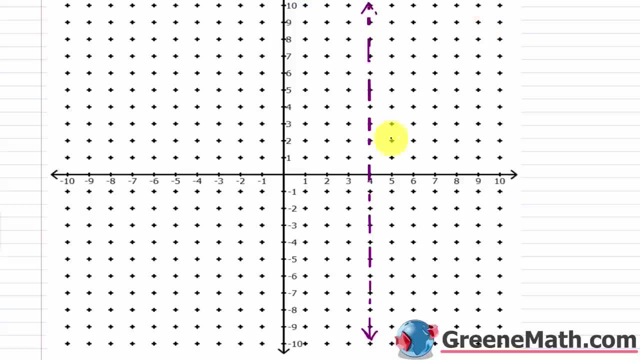 Okay, so that's a broken up or dashed line. Again, just do what I'm doing here. I'm just going to draw a vertical line. Okay, so that's a broken up or dashed line. Again, just do what I'm doing here. I'm just going 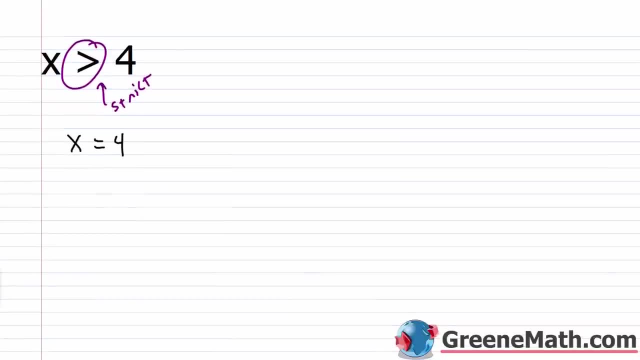 enough to where your teacher can tell what you're doing. And then x is greater than 4. 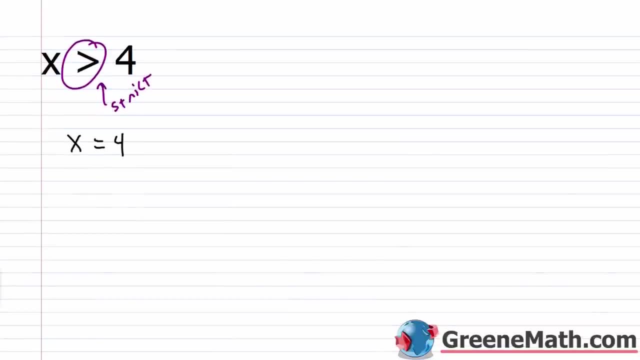 So greater than in terms of the x-axis means you're going to the right. Remember, if you're increasing on the x-axis, you're going to the right. If you're decreasing, you're going to the left. So if it's a greater than, you're shading to the right. So I want to shade in this direction now. 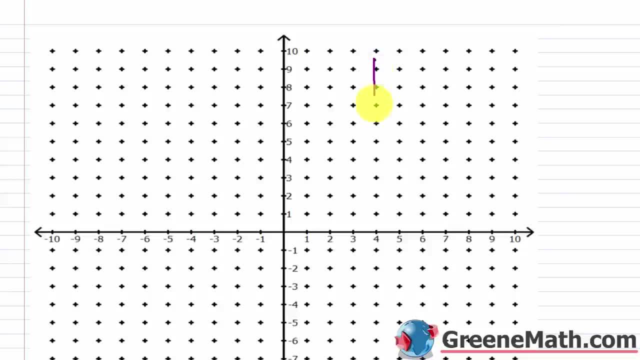 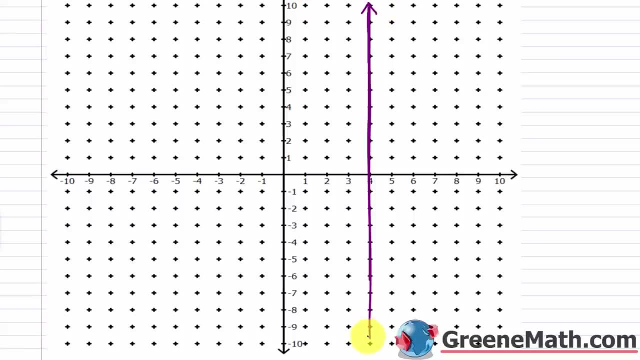 So I've got to kind of break it up or make it dashed. And now I'm going to take my eraser. just take chunks out of it. Okay, so that's a broken up or dashed line Again. just do enough to where you're. 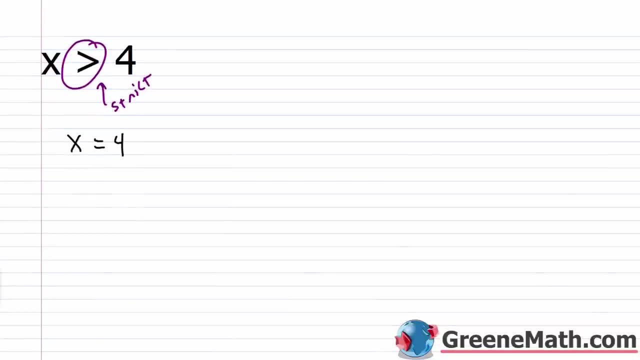 the teacher can tell what you're doing. And then x is greater than four. So greater than in terms of the x-axis means you're going to the right. Remember, if you're increasing on the x-axis, you're going to the right. 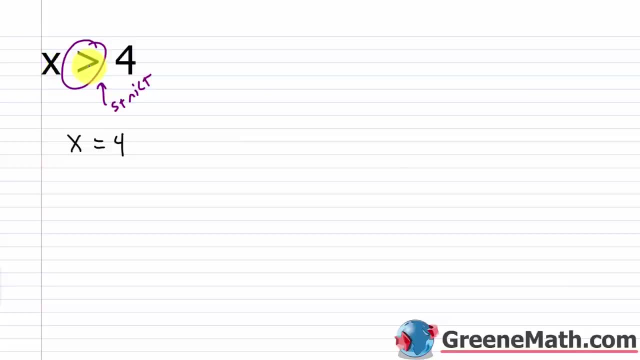 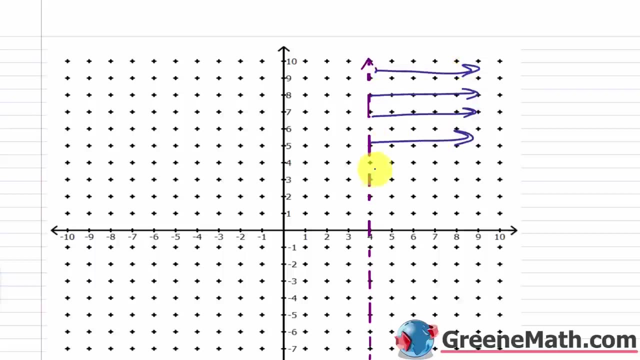 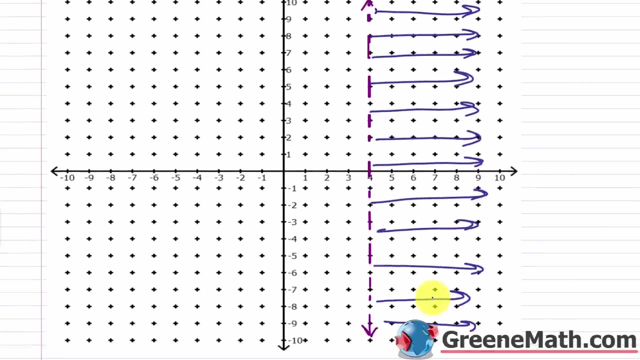 If you're decreasing, you're going to the left. So if it's a greater than you're shading to the right. So I want to shade in this direction now. Okay, Because again, any x-value in this direction is greater than the value of four. 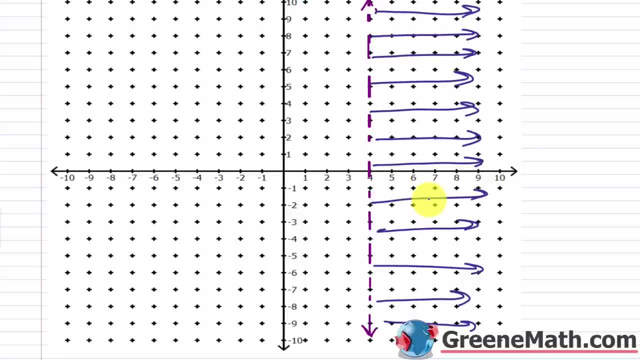 If I pick an x-value of six, it doesn't matter what y is. that value for x is greater than four. So anything to the right of four is going to work. That's why we shade all this over to the right. Hello and welcome to Algebra 1, Lesson 20.. 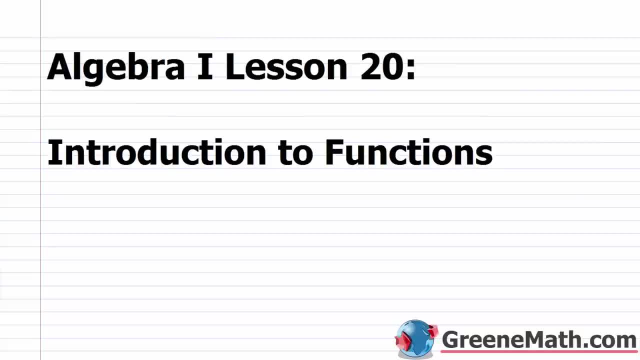 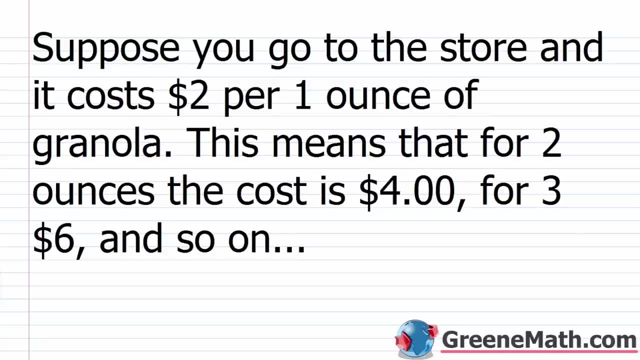 In this video we're going to have an introduction to functions. So for most of you in Algebra 1, you've never seen or heard about functions before. I can tell you that it's a topic that does confuse a lot of students. 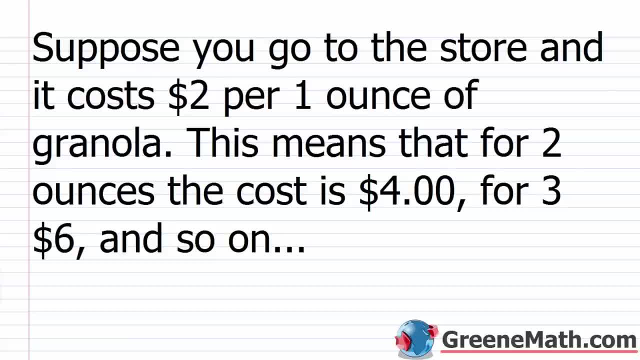 but you really don't focus a lot on it in Algebra 1.. You kind of briefly talk about it in your chapter on linear equations in two variables And then in most cases you won't see it again until Algebra 2.. So if you don't get it here, don't be too worried. 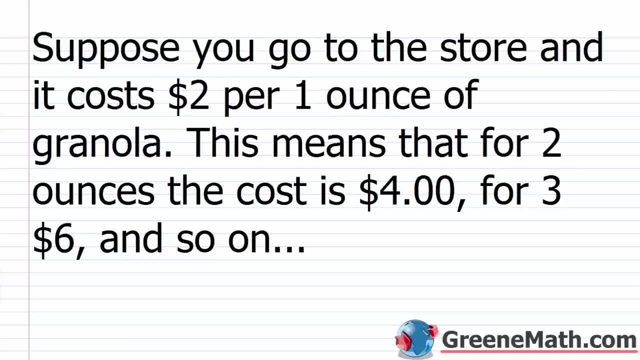 You're going to have a lot of opportunities in the future to kind of get really good at working with functions. All right, So let's start out with a basic scenario. So I want you to suppose you go to the store and it costs $2.. 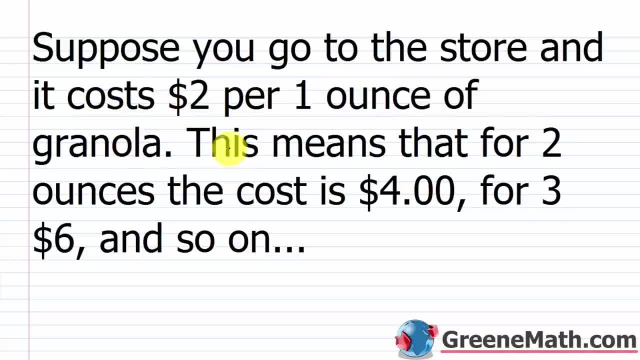 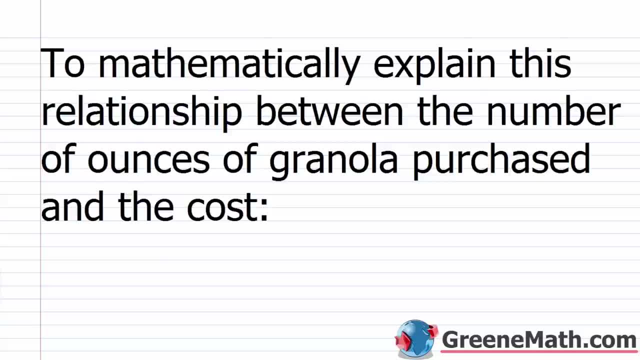 $2 per one ounce of granola. So this means for two ounces the cost is $4,, for three $6, and so on. To mathematically explain this relationship between the number of ounces of granola purchase and the cost, we could set up a little equation, right. 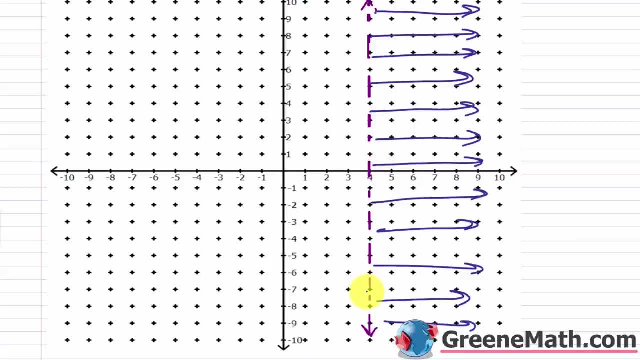 Because again, any x value in this direction is greater than the value of 4. If I pick an x value of 6, it doesn't matter what y is, that value for x is greater than 4. So anything to the right of 4 is going to work. That's why we shade all this over to the right. 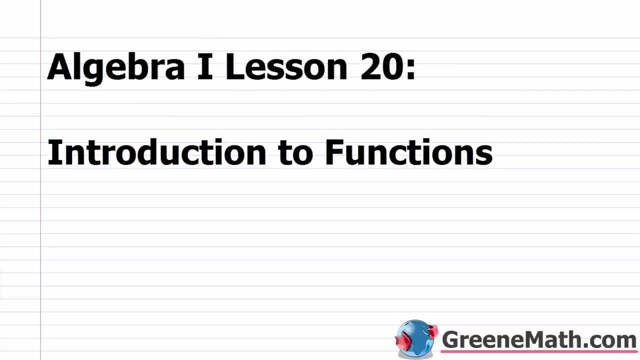 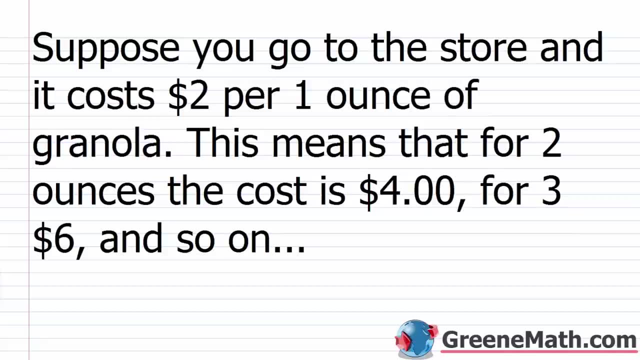 Hello, and welcome to Algebra 1 Lesson 20. In this video, we're going to have an introduction to functions. So for most of you in Algebra 1, you've never seen or heard about functions before. I can tell you that it's a tough one. I can tell you that it's a tough one. I can tell you that it's a topic that does confuse a lot of students, but you really don't focus a lot on it in Algebra 1. You kind of briefly talk about it in your chapter on linear equations in two variables, and then in most cases, you won't see it again until Algebra 2. So if you don't get it here, don't be too worried. You're going to have a lot of opportunities in the future to kind of get really good at working with functions. 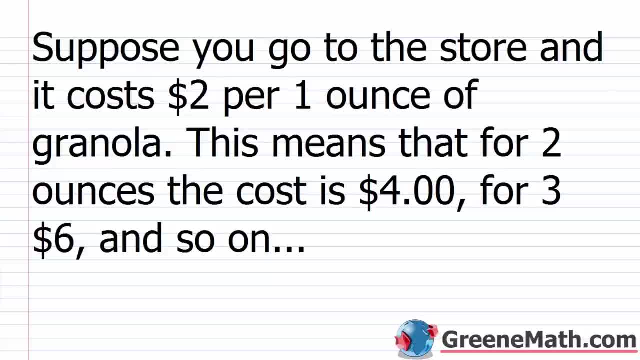 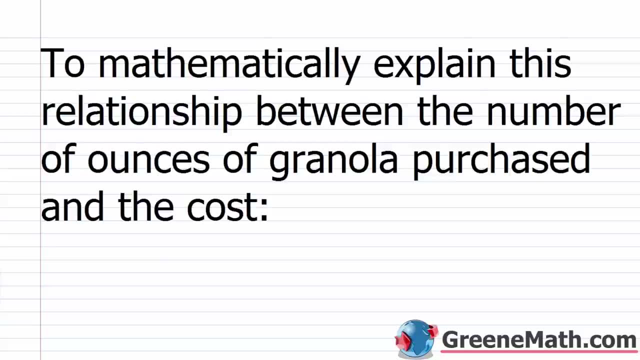 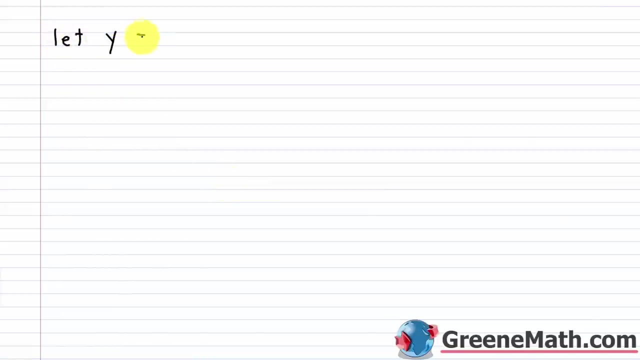 All right, so let's start out with a basic scenario. So I want you to suppose you go to the store and it costs $2. $2 per one ounce of granola. So this means for two ounces, the cost is $4, for three, $6, and so on. To mathematically explain this relationship between the number of ounces of granola purchased and the cost, we could set up a little equation, right? We could set up a linear equation in two variables. So let's let Y be equal to the total cost in dollars. And we're going to let X be equal to the number of ounces of granola that's purchased. So how would we take these two variables and set up an equation that describes our situation? Well, I know that $2, or $2 specifically, I'm going to leave off the dollar symbol. I know that $2 is the cost of granola. So I'm going to set up a linear equation to represent the cost per ounce of granola. So this is the cost per ounce. And I know that X is representing the number of ounces of granola purchased. So if I multiply the two together, if I take two, the cost per ounce, and I multiply it by X, the number of ounces of granola purchased, that's going to give me the total cost, which is Y. This is the total cost in dollars. 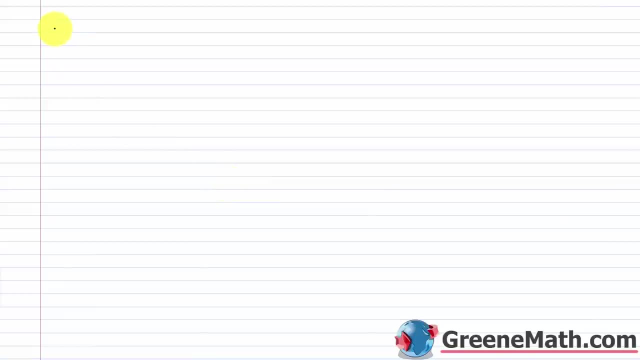 We could set up a linear equation in two variables. So let's let y be equal to the total cost in dollars, And we're going to let x be equal to the number of ounces of granola that's purchased. So how would we take these two variables and set up an equation that describes our situation? 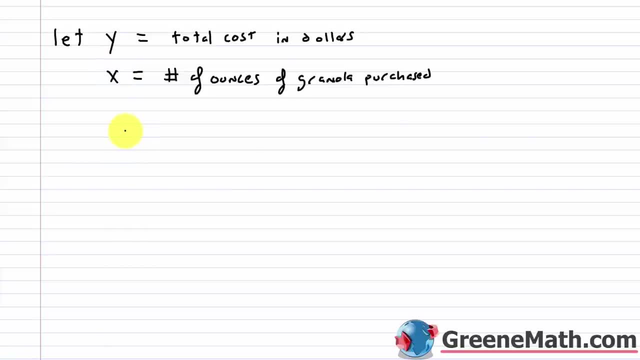 Well, I know that 2, or $2- specifically, I'm going to leave off the dollar symbol- I know that 2 is the cost per ounce of granola, So this is the cost per ounce, And I know that x is representing the number of ounces of granola purchase. 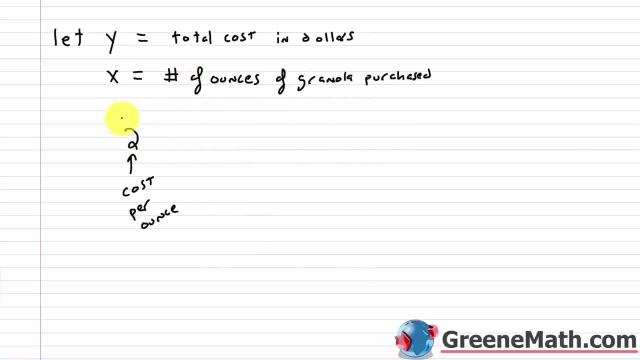 So if I multiply the two together, if I take 2, the cost per ounce and I multiply by x the number of ounces of granola purchase, that's going to give me the total cost, which is y. This is the total cost in dollars. 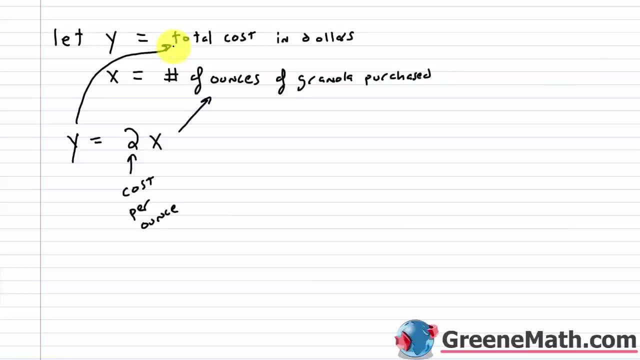 So there's an equation to write. So there's an equation to write. So there's an equation to write And I'm going to represent the scenario that I just gave you Now the ordered pairs that satisfy this equation. So, for example, one ordered pair would be 0,0.. 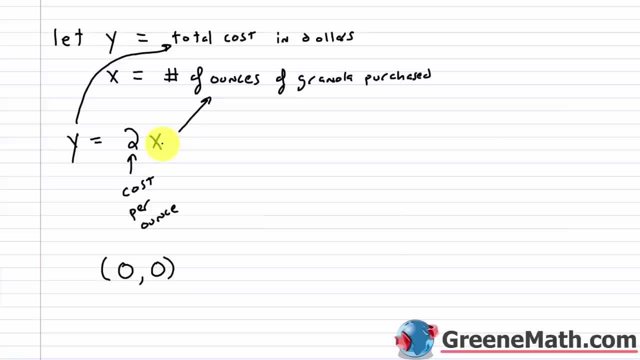 I plug in a 0 for x, meaning I don't buy any ounces of granola. I would get a 0 for y: I didn't buy any ounces of granola, I don't spend any money. Another one would be 1,2.. 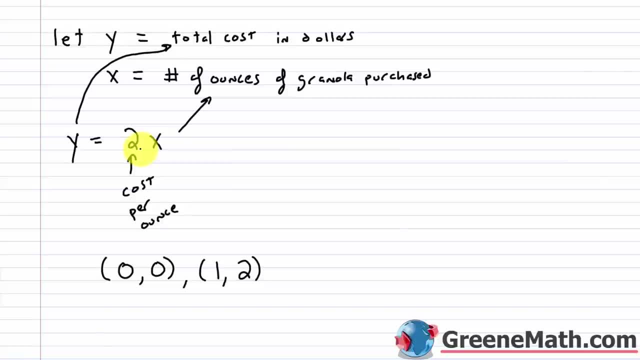 I buy 1 ounce of granola, I spend $2. dollars. another one would be two comma four: i buy two ounces of granola, i spend four dollars. right, so on and so forth. so i can kind of put a comma here and three dots, because this pattern. 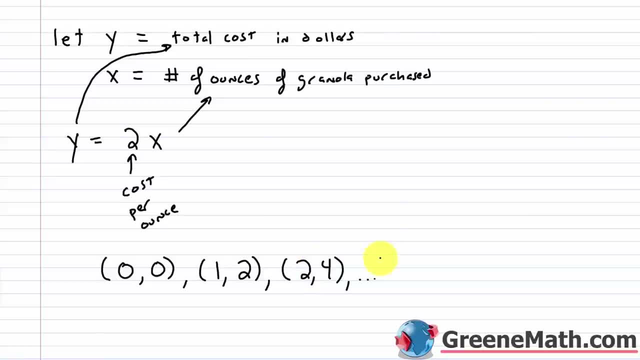 would continue forever. after two for an x value, i would get three, and i would just double it to get my answer. three times two is six, then four times two is eight, then five times two is ten, so on and so forth. if i plugged in 27 for x, i just multiply it by two and get 54, my y value. 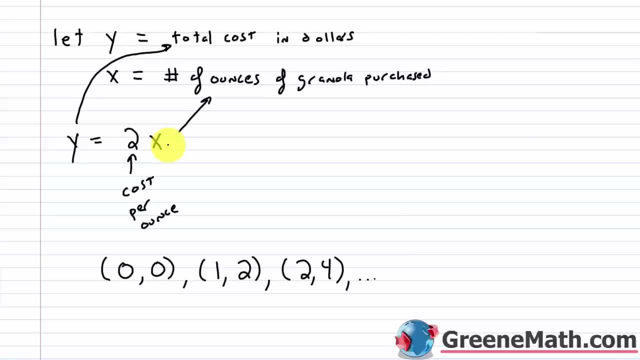 one thing that you might not have noticed here is that there's a restriction on x, and a lot of times when we work with these real world problems, you have restrictions. why is there a restriction on x? can you think about what x can't be equal to? well, x specifically can't be negative. it can be. 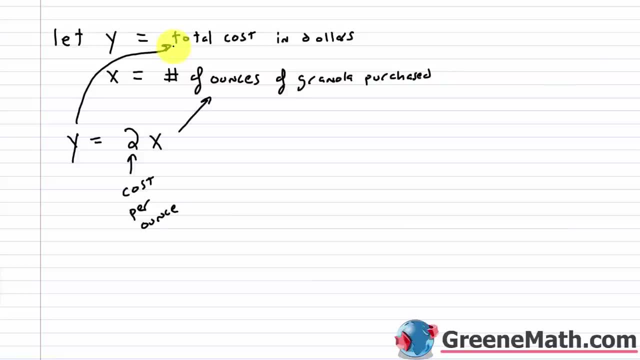 So there's an equation to represent the total cost in dollars. So let's say I want to take $4. the scenario that I just gave you now the ordered pairs that satisfy this equation so for example one ordered pair would be 0 comma 0 I plug in a 0 for X meaning I don't buy any ounces of granola I would get a 0 for Y I didn't buy any ounces of granola I don't spend any money another one would be 1 comma 2 I buy one ounce of granola I spend $2 another one would be 2 comma 4 I buy 2 ounces of granola I spend $4 right so on and so forth so I can kind of put a comma here and three dots because this pattern would continue forever after 2 for an X value I would get 3 and I would just double it to get my answer 3 times 2 is 6 then 4 times 2 is 8 then 5 times 2 is 10 so on and so forth if I plugged in 27 for X I just multiply it by 7 and so on and so forth then I would get 3 and so forth then I would multiply it by 2 and get 54 my Y value one thing that you might not have noticed here is that there's a restriction on X and a lot of times when we work with these real-world problems you have restrictions why is there a 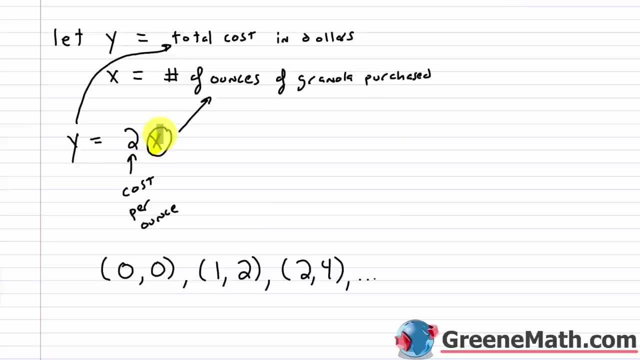 restriction on X can you think about what X can't be equal to well X specifically can't be negative it can be 0 or it can be positive so X is greater than or equal to 0 here specifically because I can't walk into a grocery store and say hey I'd like to go to a grocery store and say hey I'd like to buy negative 18 ounces of granola all right maybe that's you selling granola or something like that but you know we're not going to get into any complicated scenarios or thought processes like that we're just gonna say that hey we can only buy zero ounces of granola or some positive amount so there's a restriction here there's a restriction and we're going to talk a lot about this moving forward where we're limiting a variable to certain values and In this case, we're gonna say, hey, it can only be zero or some positive value. 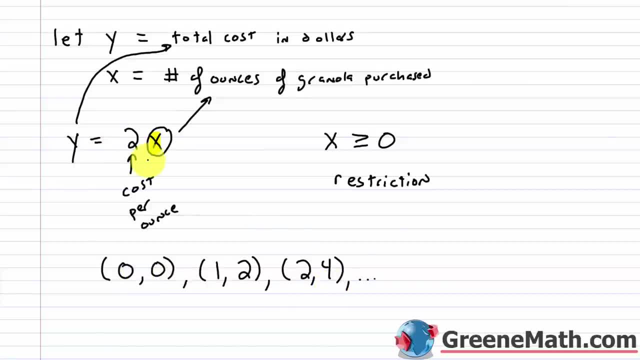 So the ordered pairs here that satisfy this equation have a special name when we're talking about functions. 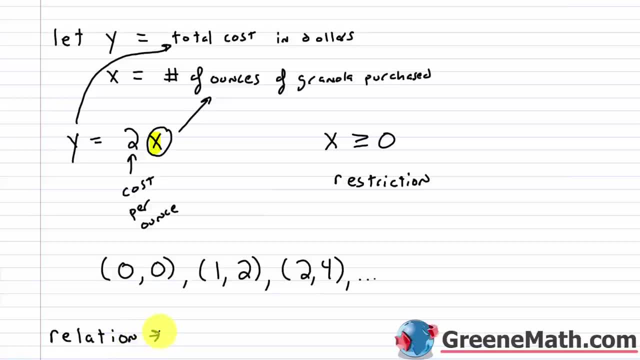 This is definitely a definition you wanna write down. It's something you're gonna talk about when you study functions. 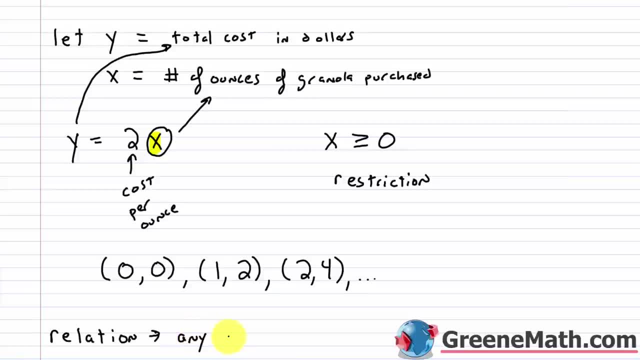 So a relation is just any set, any set of ordered pairs. 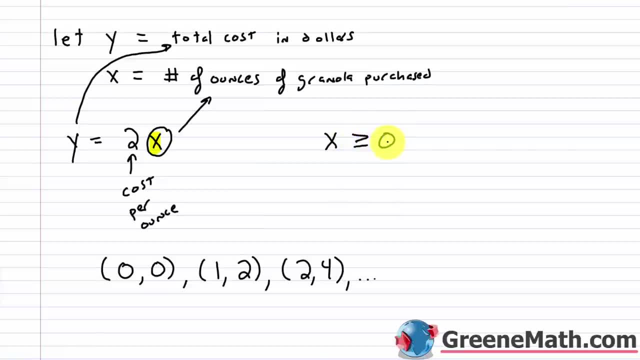 zero, or it can be positive, so x is greater than or equal to zero here, specifically because i can't walk into a grocery store and say: hey, i'd like to buy negative 18 ounces of granola. right, maybe that's one of the most important things in the world, so i can't buy negative 18 ounces of granola. 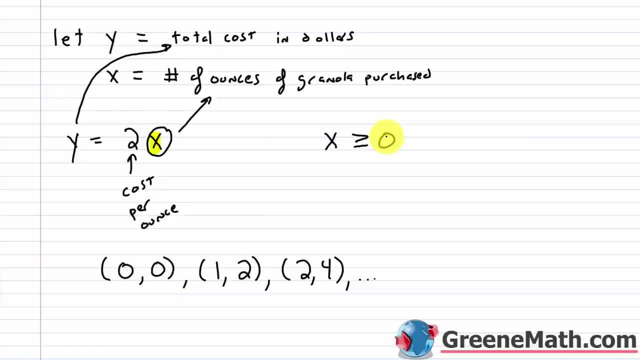 right, maybe that's one of the most important things in the world, so i can't buy negative 18 ounces of you selling granola or something like that. But you know we're not going to get into any complicated scenarios or thought processes like that, We're just going to say that. 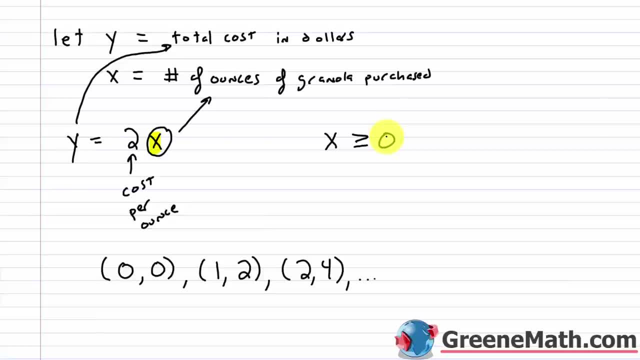 hey, we can only buy zero ounces of granola or some positive amount. So there's a restriction here. There's a restriction- And we're going to talk a lot about this moving forward- where we're limiting a variable to certain values. In this case, we're going to say, hey, it can only be zero or some positive value. 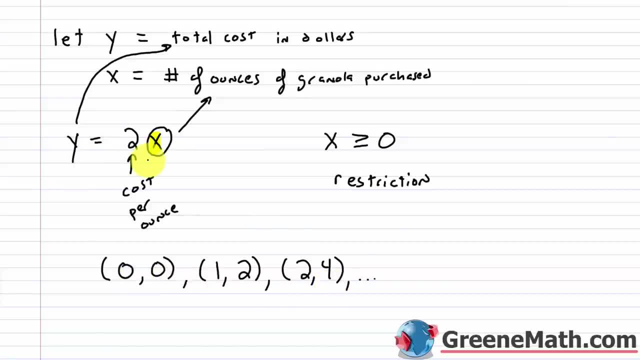 So the ordered pairs here that satisfy this equation have a special name. when we're talking about functions, They're known as a relation. They're known as a relation. This is definitely a definition you want to write down. It's something you're going to. 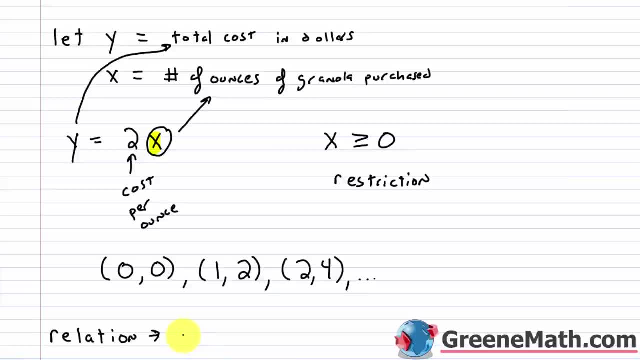 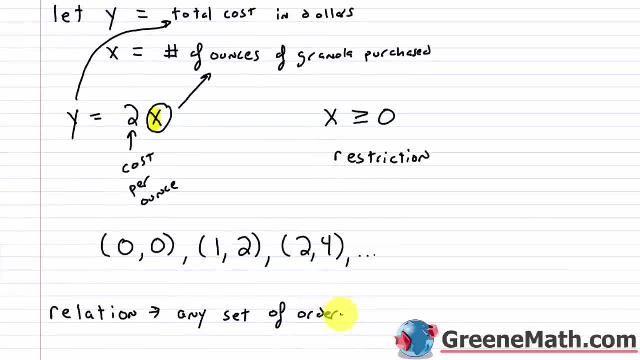 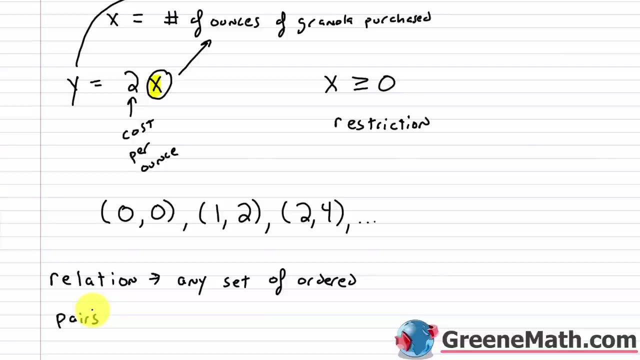 talk about when you study functions. So a relation is just any set, any set of ordered pairs, And we haven't really talked about what a set is either. We'll talk a lot about sets in Algebra 2. But for right now, just understand that a set is a collection of things. 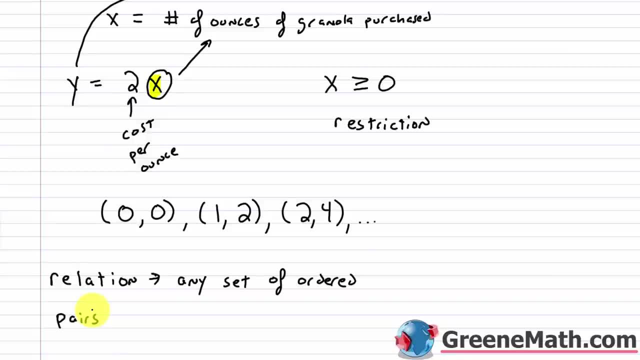 And when we work with sets, we put the elements of a set- and that's what's contained in a set- inside of what's known as set braces. So, for example, here with these ordered pairs, I'll put them inside of set braces. 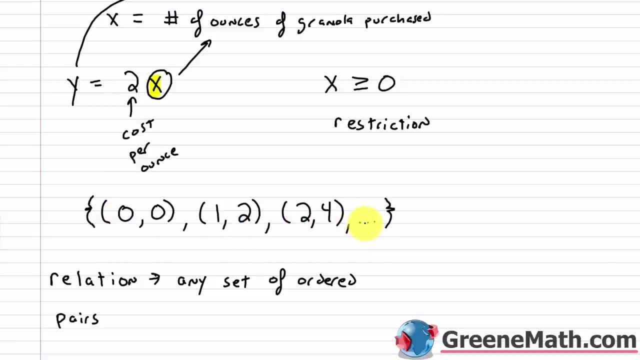 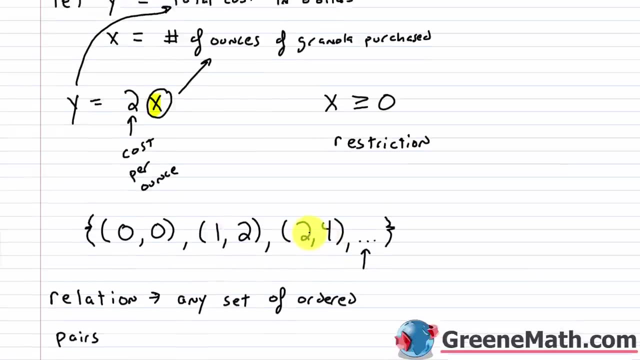 Okay, So this would be the set of ordered pairs that satisfy this equation, And I can't possibly list all of the ordered pairs, So again I have the three dots to say that the pattern here, where I increase x by 1 and y increases by 2, continues forever and ever, and ever. 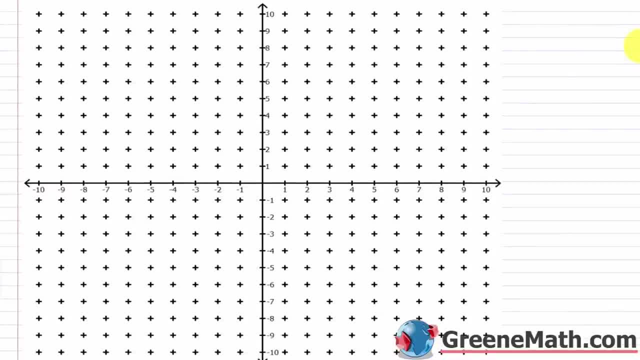 Now one thing I want to do really quickly is just graph this equation: y equals 2x, where again x is greater than or equal to 0. So I know the y-intercept: it occurs at 0, 0, right, It occurs at the origin. 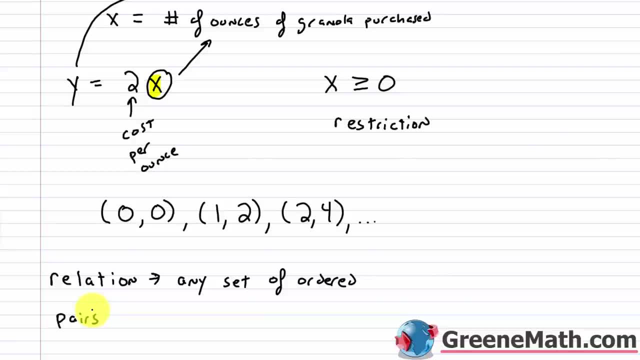 And we haven't really talked about what a set is either. We'll talk a lot about sets in algebra two, but for right now, just understand that a set is a collection of things, okay? And when we work with sets, we put the elements of a set, and that's what's contained in a set, inside of what's known as set braces. So for example, here with these ordered pairs, I'll put them inside of set braces. 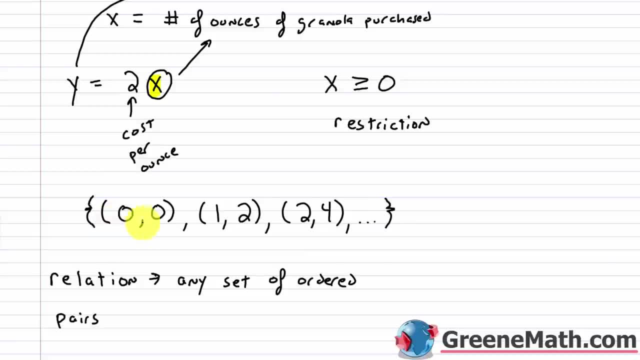 Okay? So this would be the set of ordered pairs 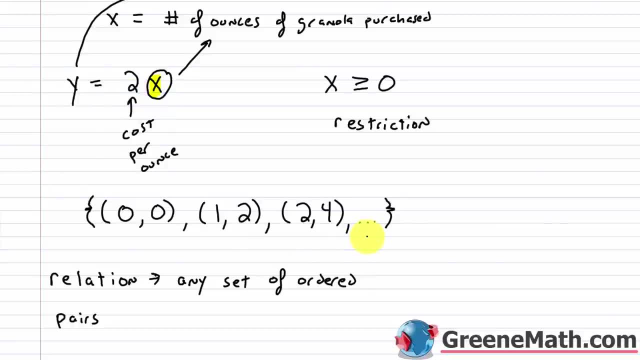 that satisfy this equation. And I can't possibly list all of the ordered pairs. So again, I have the three dots to say that the pattern here where I increase x by one and y increases by two continues forever and ever and ever. 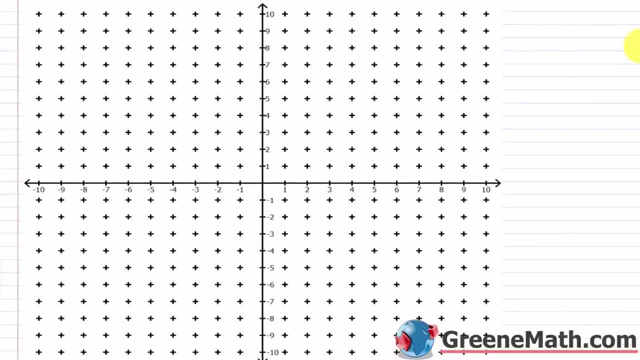 Now, one thing I wanna do really quickly is just graph this equation y equals two x, where again, x is greater than or equal to zero. 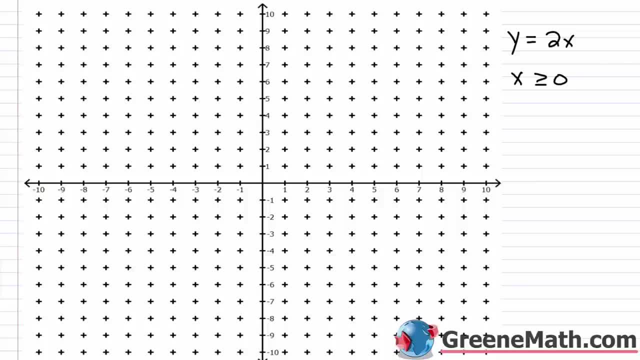 So I know the y intercept occurs at zero comma zero, right? It occurs at the origin. 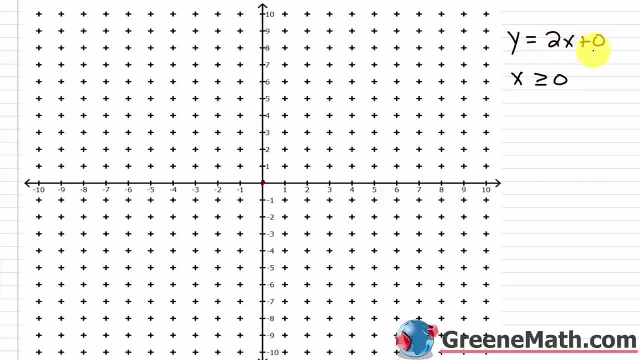 This is in slope intercept form. I could put plus zero behind this if I wanted to, or you could just realize, again, that's a line that goes through the origin. 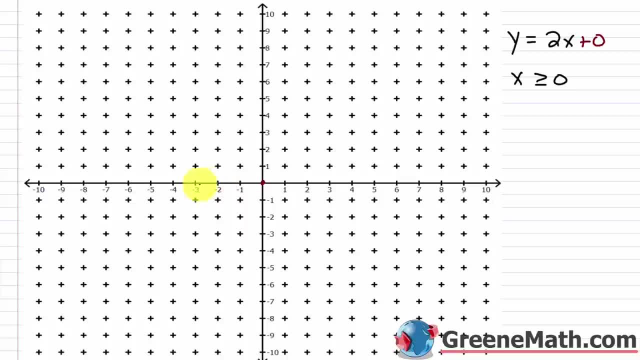 Now, I can't have any points that correspond with an x value that's to the left of zero. So I'm only gonna plot points up here, because again, x has to be greater than or equal to zero. 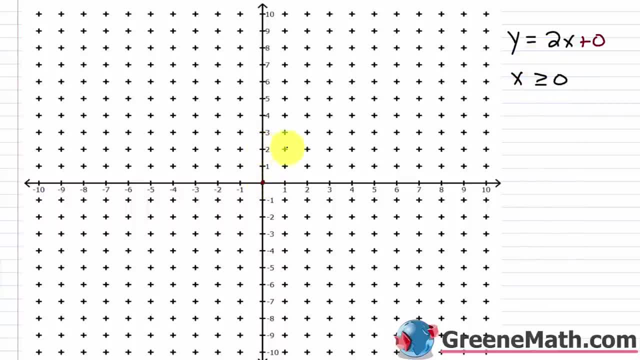 So if I use my slope, I'd go up two, I go up one, two, and over one, up two and over one, up two and over one. So let's graph this guy. 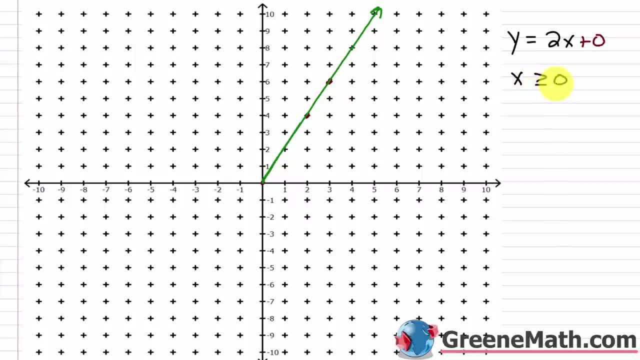 So this would be y equals two x with x is greater than or equal to zero. 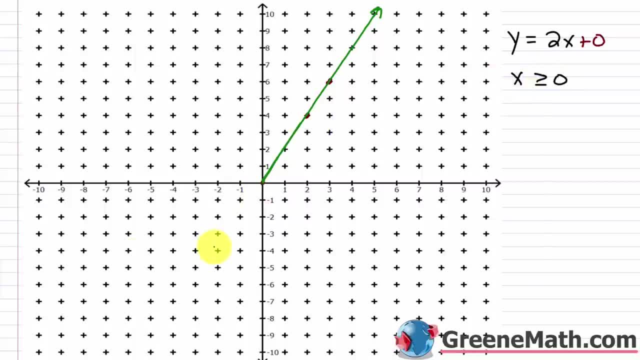 Again, notice how we don't have anything down here like we normally would. 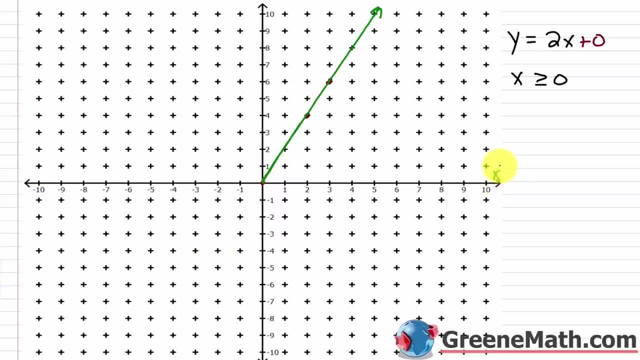 And this shows the relationship between, again, the x-axis is telling us how many ounces of granola that we're purchasing. 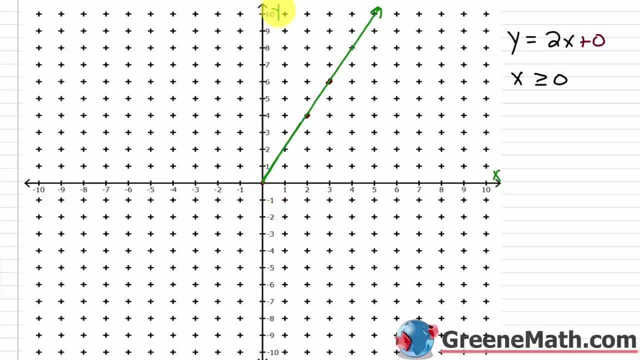 The y-axis is telling us how much it costs in dollars. So in other words, if I buy one ounce of granola, it's gonna cost me $2. 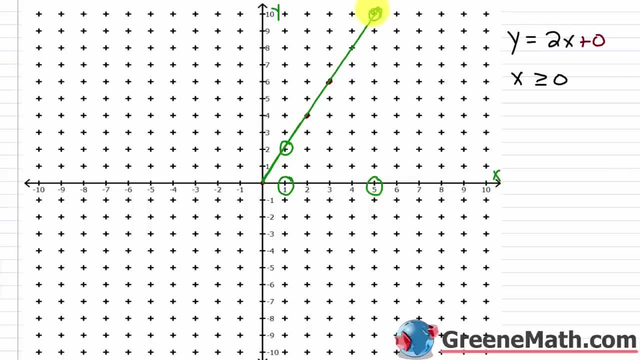 If I buy five ounces of granola, it's gonna cost me $10. Right, so on and so forth. 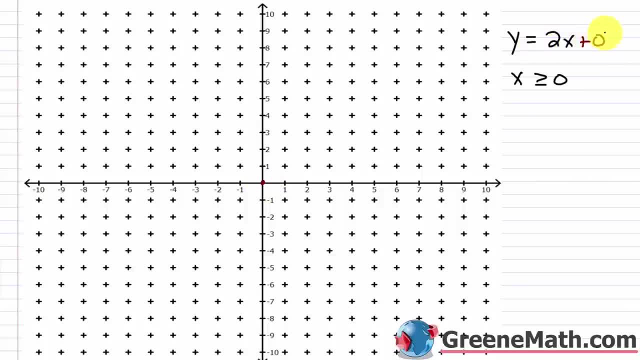 This is in slope-intercept form. I could put plus 0 behind this if I wanted to, Or you could just realize again. that's a line that goes through the origin. Now I can't have any points that correspond with an x value, that's. 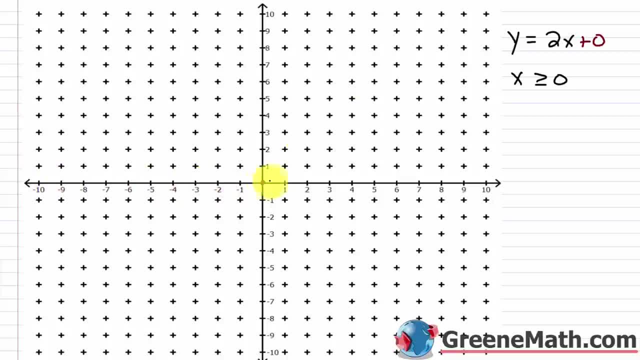 to the left of 0. So I'm only gonna plot points up here because again, x has to be greater than or equal to 0. So if I use my slope I'd go up 2,, I go up 1,, 2, and over 1.. 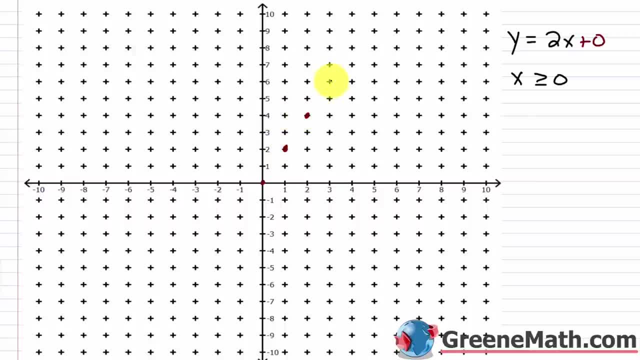 Up 2, and over 1.. Up 2, and over 1.. So let's graph this guy. So this would be: y equals 2x, with x is greater than or equal to 0.. Again, notice how we don't have anything down here like we normally would. 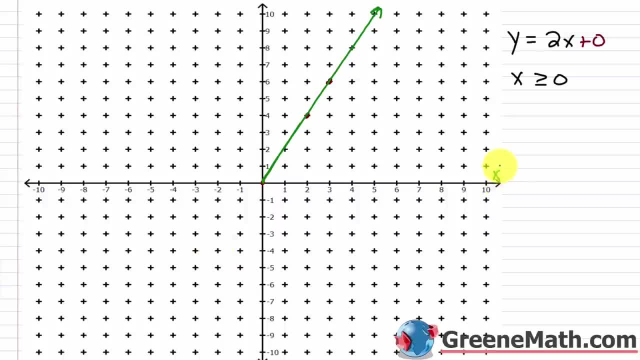 And this shows the relationship between. again, the x-axis is telling us how many ounces of granola that we're purchasing. The y-axis is telling us how much it costs in dollars. So in other words, if I buy 1 ounce of granola, it's gonna cost me $2.. 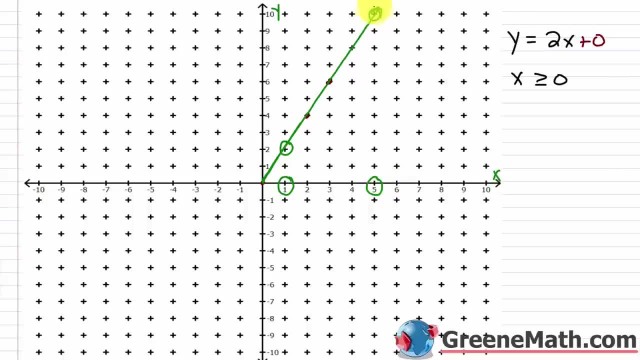 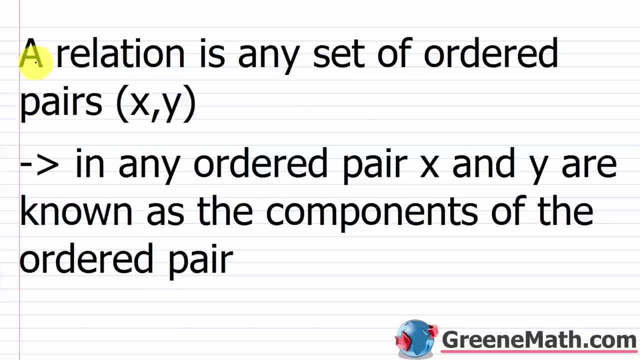 If I buy 5 ounces of granola, it's gonna cost me $10.. Right, so on and so forth. Alright, so let's talk a little bit more about some basic vocabulary. So we already know that a relation is any set of ordered pairs, and the ordered pairs are again x, y. 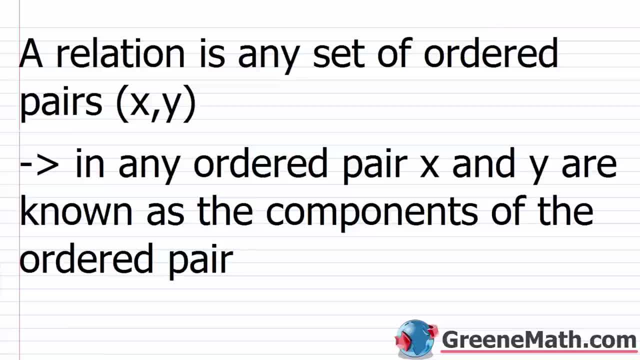 So, in any ordered pair, x and y are known as the components, The components of the ordered pair, Something that you want to write down because, again, when you start talking about functions, you get a lot of these new kind of definitions that are gonna pop up. 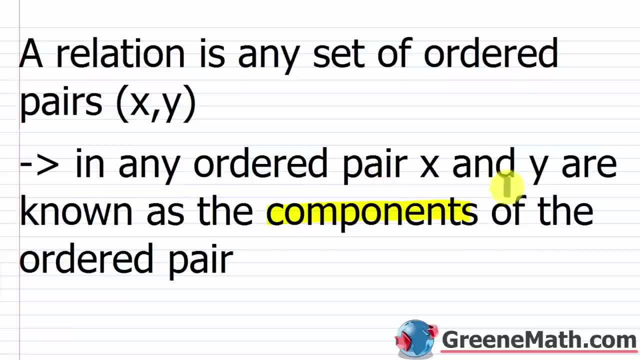 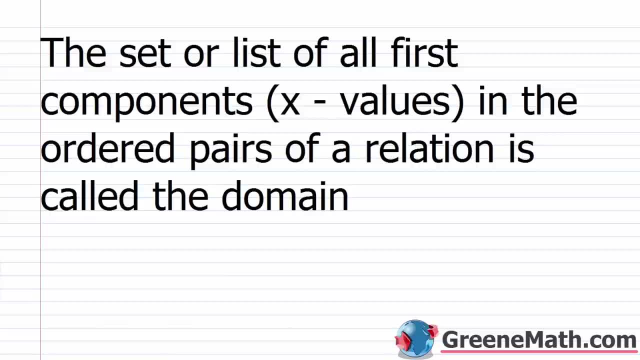 It might be put on your test. So just write down again: in any ordered pair, x and y are known as the components of the ordered pair. Now, highly important here, The set or the list of all first components. so basically they're saying x values. 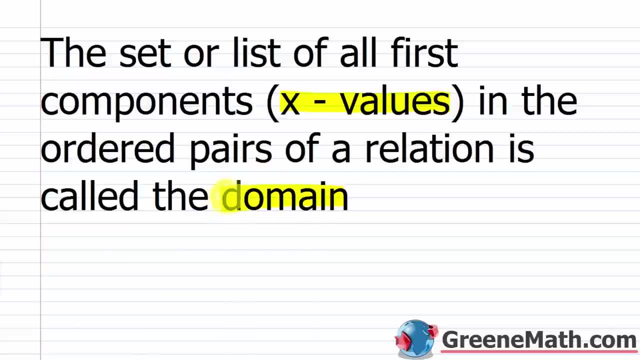 in the ordered pairs of relation is called the domain. You're gonna hear a lot about the domain moving forward. What's the domain? Find the domain Right, so on and so forth. Now the set or the list of all second components. again, these would be the y values. 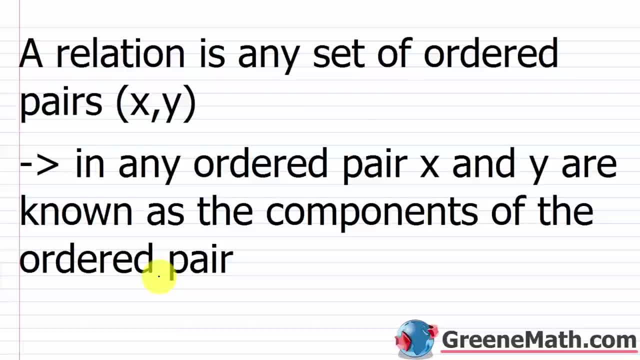 Alright, so let's talk a little bit more about some basic vocabulary. So we already know that a relation is any set of ordered pairs. 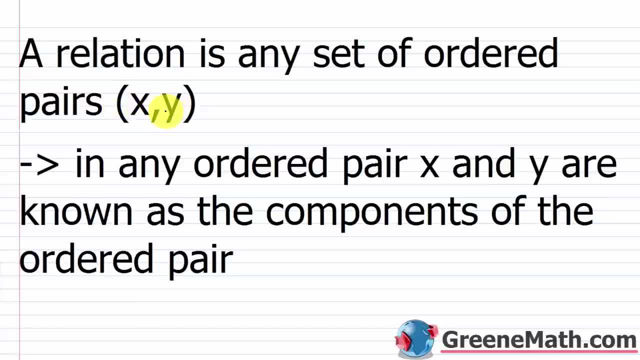 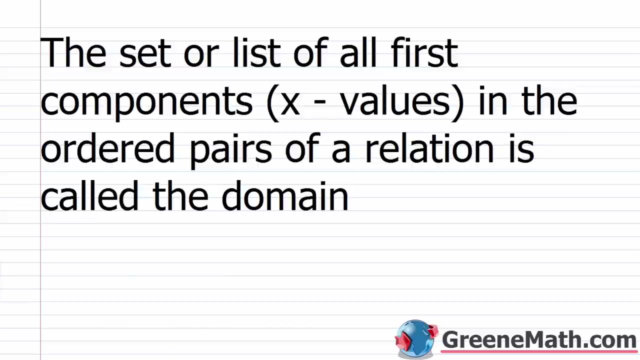 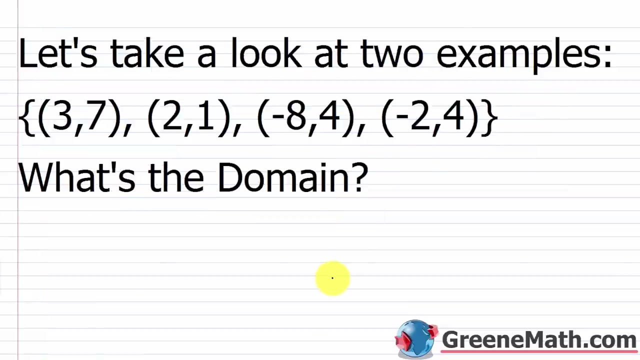 And the ordered pairs are, again, x comma y. So in any ordered pair, x and y known as the components the components of the ordered pair something that you want to write down because again when you start talking about functions you get a lot of these new kind of definitions that are going to pop up it might be put on your test so just write down again in any ordered pair x and y are known as the components of the ordered pair now highly important here the set or the list of all first components so basically they're saying x values in the ordered pairs of relation is called the domain you're going to hear a lot about the domain moving forward what's the domain find the domain right so on and so forth now the set or the list of all second components again these would be the y values and the ordered pairs of relation is called the range okay so you might get questions that say what's the domain of this function well you're looking for the set or the list of all positive x values you might get a question that says hey what's the range of this function well you're looking for again the list or the set of all possible y values alright so let's take a look at some basic examples right now and we 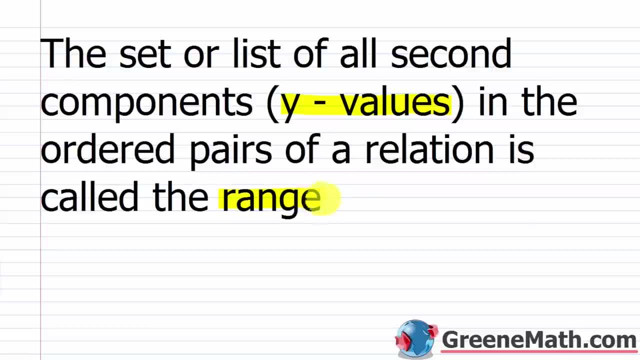 in the ordered pairs of relation is called the range. Okay, so you might get questions that say: what's the domain of this function? Well, you're looking for the set or the list of all possible x values. Okay, You might get a question that says, hey, what's the range of this function? 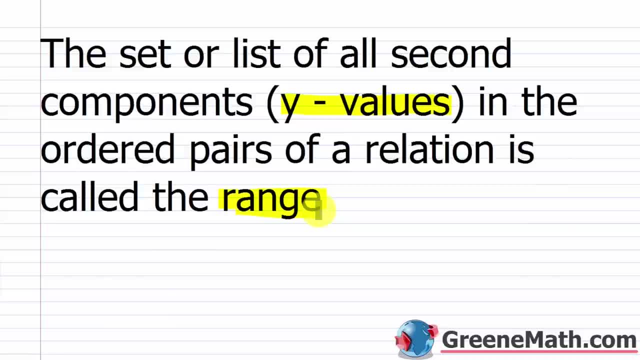 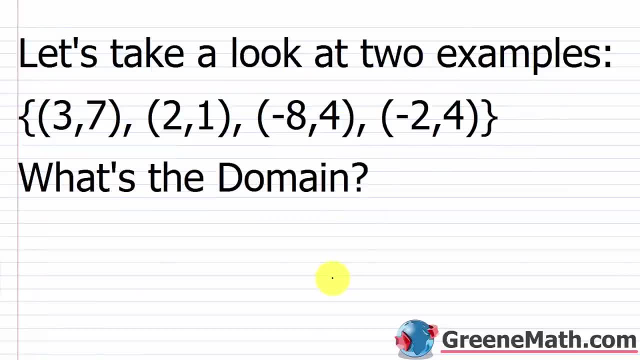 Well, you're looking for again the list or the set of all possible y values. All right, so let's take a look at some basic examples right now- And we have more stuff to explain. We haven't even gotten to functions yet. 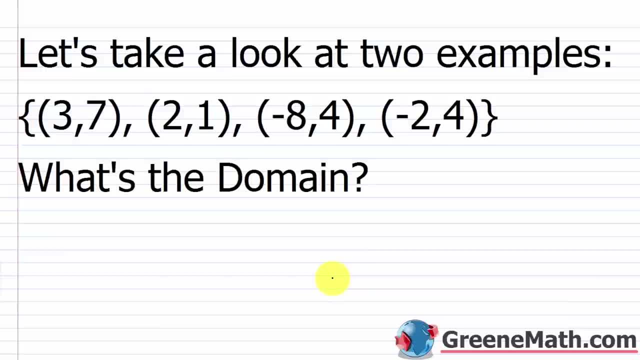 Right now we're just working with some relations and we're getting down some basic vocabulary. So let's take a look at two examples. We have this set of ordered pairs And again we have a set of ordered pairs. It makes up a relation. 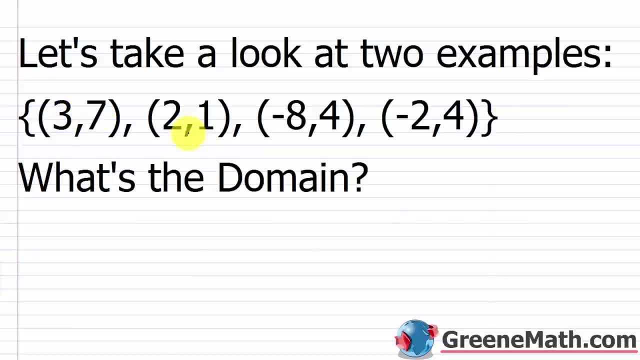 So the first ordered pair is three comma seven, The second one is two comma one, The third one is negative eight comma four And the fourth one is negative two comma four. Now it says what is the domain. So the domain again is the set of all first components. 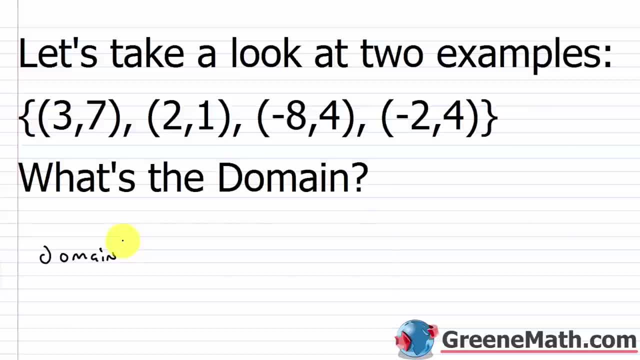 And again, that's kind of very textbooky, right, You want to say the set of all first components, meaning the set of all x's. So what are the set of all x's? What are the x values in this relation? 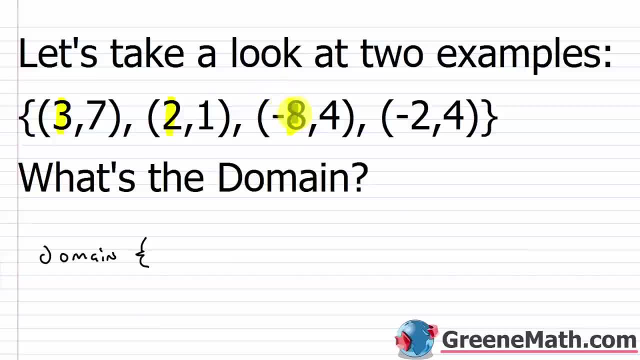 Well, it's everything that occurs first. right, These are your x values. That's all you're looking for, if it asks you for the domain. So it's the number three, It's the number two, It's the number negative eight. 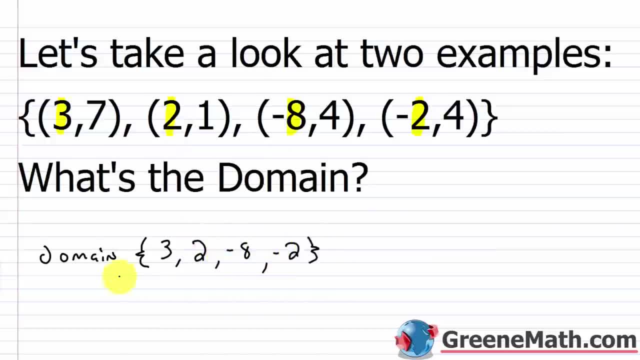 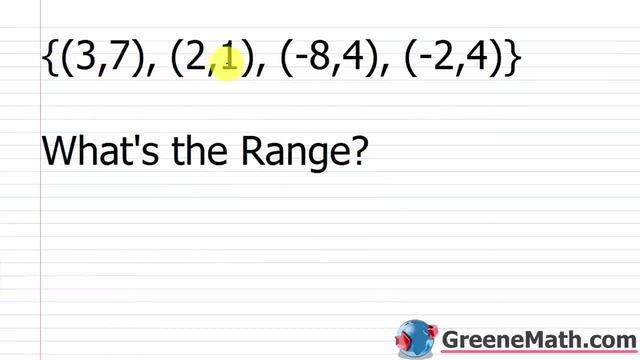 And it's the number negative two. So this is your domain, All right, so now we want to find the range. So we have this same relation: Three comma seven, two comma one, negative eight comma four and negative two comma four. 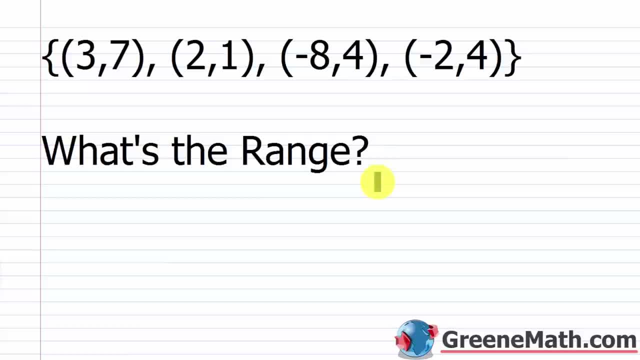 So the range is the set of all second components or y values. So seven, one, four and four. So for the range we'll have- and let me make that better- we'll have seven, we'll have one and we'll have four. 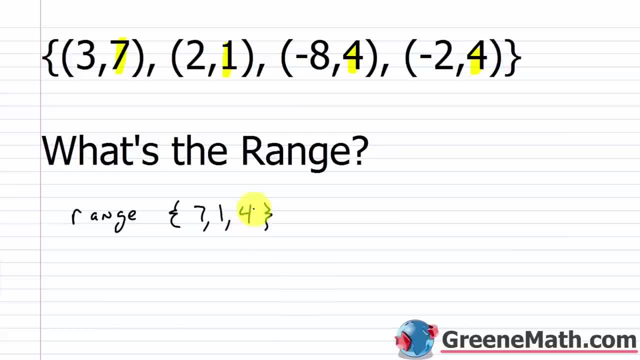 I don't need to list four twice When you're writing a set. if you already have something in there, you don't need to list it again. So just seven: one and then four. So let's take a look at another one. 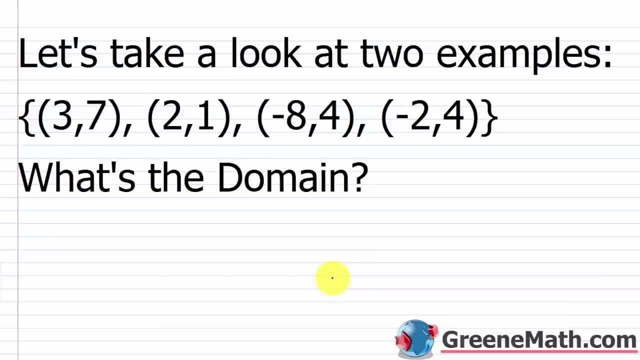 have more stuff to explain we haven't even gotten to functions yet right now we're just working with some relations and we're getting down some basic vocabulary so let's take a look at two examples we have this set of ordered pairs and again we have a set of ordered pairs it makes up a relation so the first order pair is 3 comma 7 the second one is 2 comma 1 the third one is negative 8 comma 4 and the fourth one is negative 2 comma 4 now it says what is the domain so the domain again is the set of all first components and again that's kind of very textbook II right you want to say the set of all first components and again that's kind of very textbook II right you want to say the set of all first components meaning the set of all X's so what are the X values in this relation well it's everything that occurs first right these are your X values that's all you're looking for if it asks you for the domain so it's the number 3 it's the number 2 it's the number negative 8 and it's the number negative 2 so this is your domain alright so now we want to find the range so we have the same relation 3 comma 7 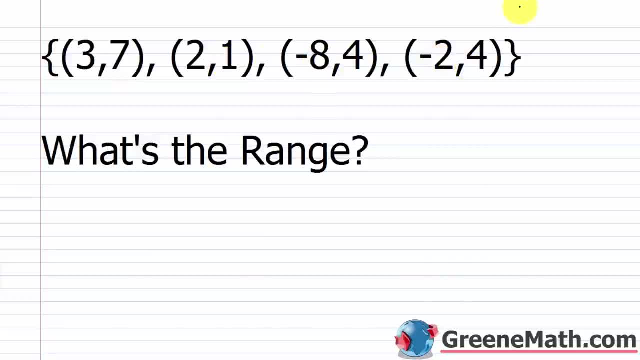 2 comma 1 negative 8 comma 4 and negative 2 comma 4 so the range is the set of all second components or Y values so 7 1 4 and 4 so for the range we'll have and let me make that better we'll have 7 we'll have 1 and we'll have 4 I don't need to list 4 twice when you're writing a set if you already have 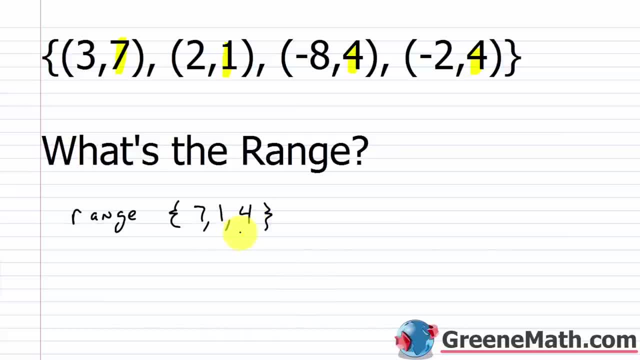 something in there you're going to want to make sure that you're going to have it you don't need to list it again so just 7 1 and then 4 so let's take a look 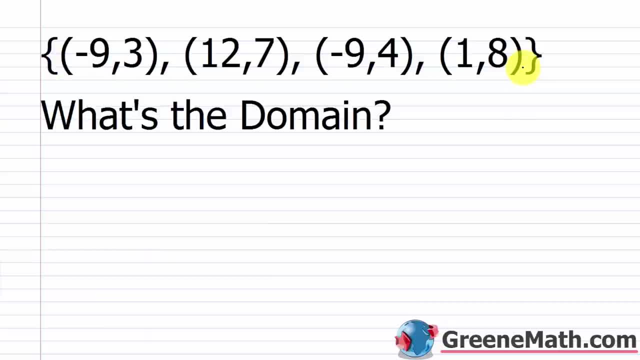 at another one we have a relation here which is made up of these four ordered pairs so we have negative 9 comma 3 12 comma 7 negative 9 comma 4 and 1 comma 8 so what's the domain again that's the set of all first components so negative 9 12 negative 9 and 1 so your domain your domain 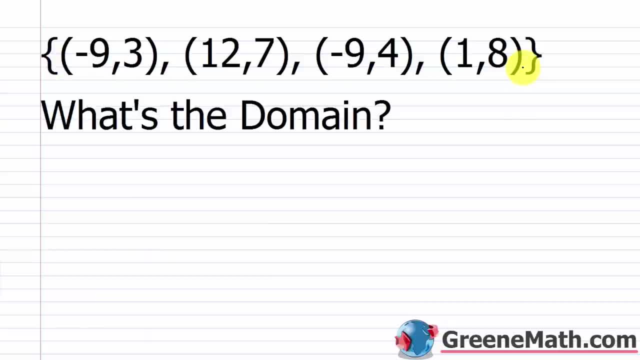 We have a relation here which is made up of these four ordered pairs. So we have negative nine comma three, twelve comma seven, negative nine comma four and one comma eight. So what's the domain? Again, that's the set of all first components. 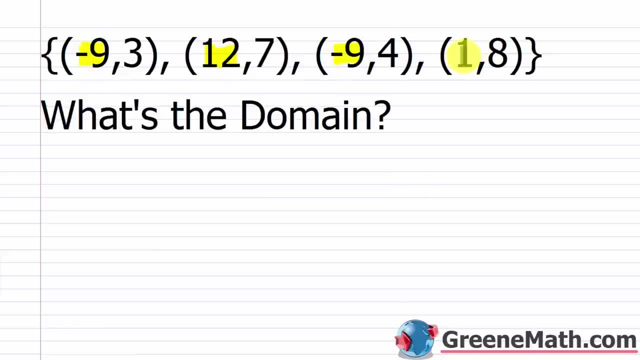 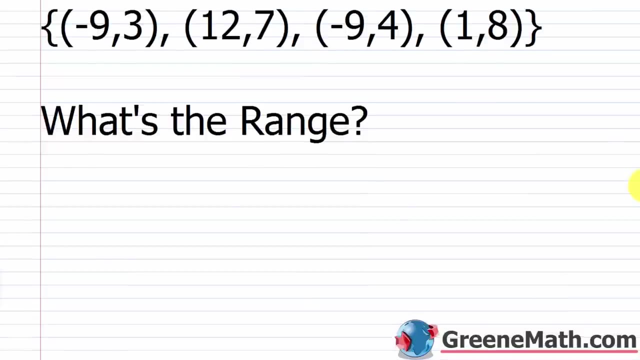 So negative nine, twelve, negative nine and one. So your domain, your domain, we've got negative nine, we've got twelve, We don't list, We don't list. negative nine again, and then we've got one, All right. so now, looking at the same relation, we want to know what's the range. 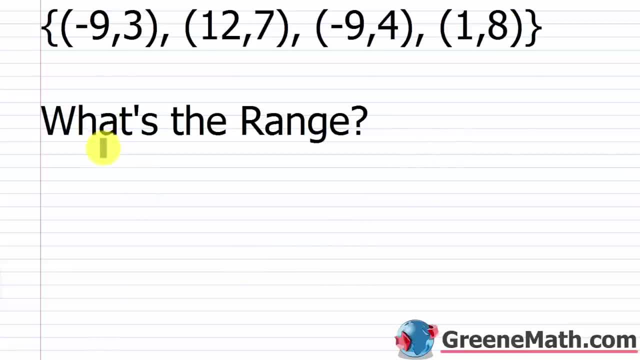 So the range again is the set of all second components, So y values. So three, seven, four and eight. So that's your range, And again let me make that better. So three, seven, four and eight. 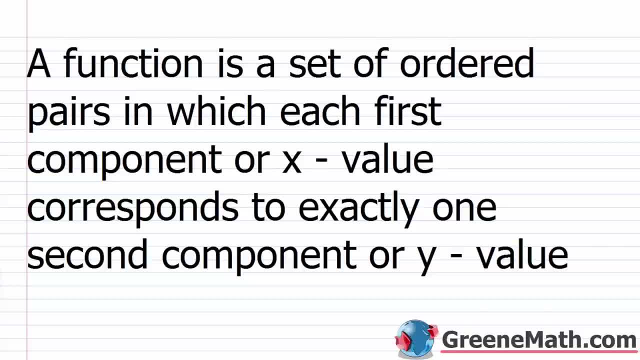 All right. so now that we've gotten some of the basic kind of the vocabulary out of the way, let's start going a little deeper and talking about functions. So a function is a set of ordered pairs in which each first component, each first component. 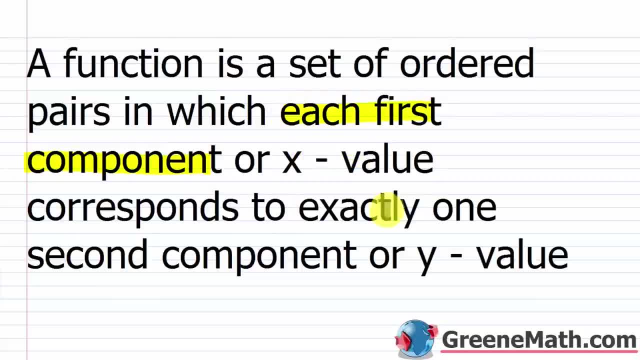 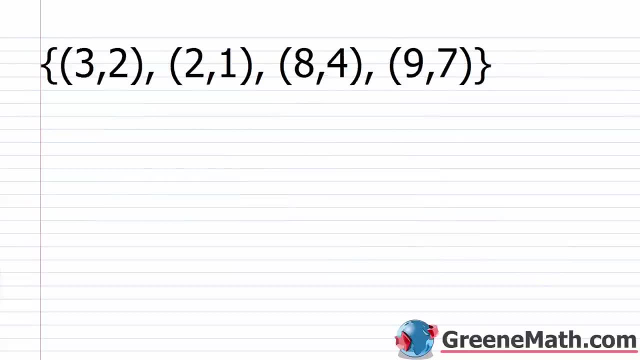 or again, that's: the x value corresponds to exactly one second component, or y value. A lot of times you're gonna hear: for each x there can be only one y. Now, in order to understand that, let's take a look at this relation here. 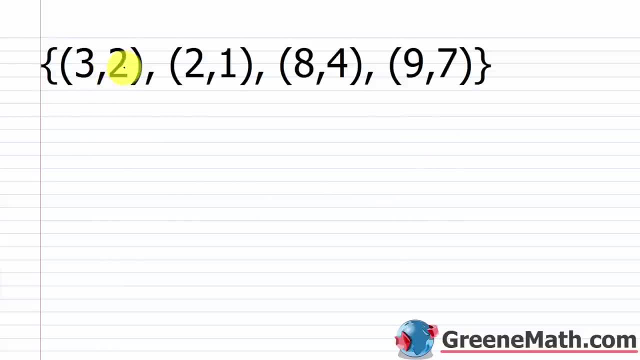 So in this relation we have the ordered pair three comma two, two comma one, eight comma four and nine comma seven. So in other words, this is going to be a function, And so not every relation is a function, but all functions are relations. 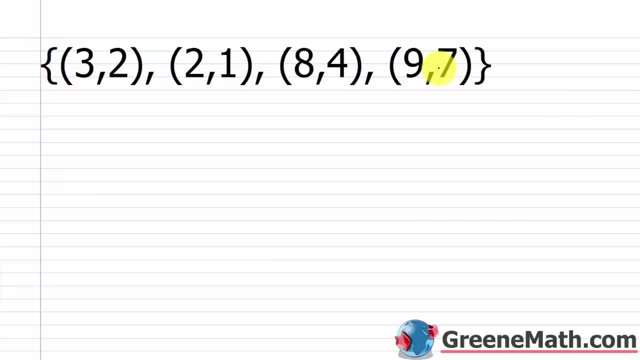 You're gonna hear that in your lecture from your teacher, or maybe your tutor will say it, or maybe you just hear me say it. But again, all functions are relations, but not all relations are functions. So if I look at each function, 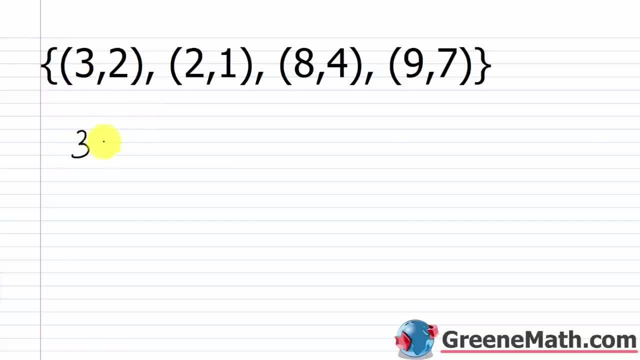 each ordered pair. here this three corresponds to two. So, in other words, I have an x value, that's three. I have a y value, that's two. Here I have an x value of two: it corresponds to a y value of one. 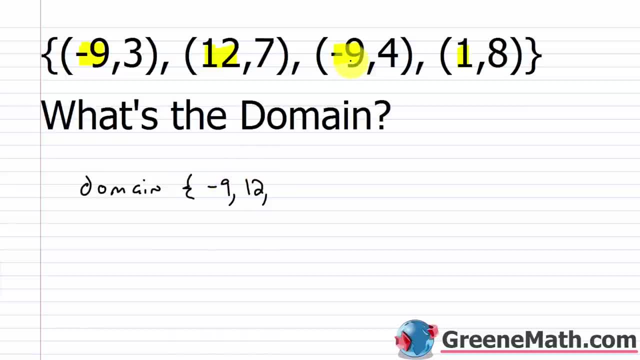 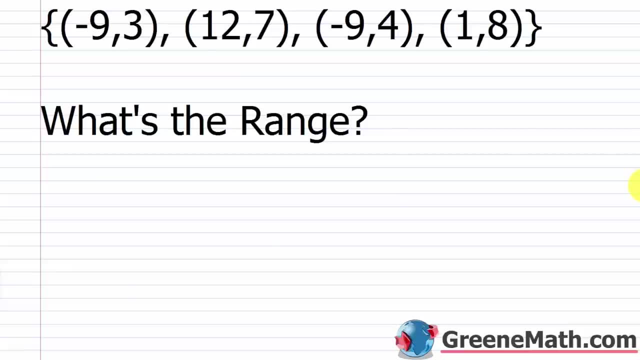 you've got negative 9 we've got negative 9 then you've got negative nine we've got negative 9 again and then we've got stu and we do that with that 4 comma 0 then we've got negative nine th w comma 1 and then we have se one and I'm gonna go up against it and I'm gonna remove that and I'm just gonna remove it because they're kimchi迡 so it's going to beouse me and all I don't want to do is 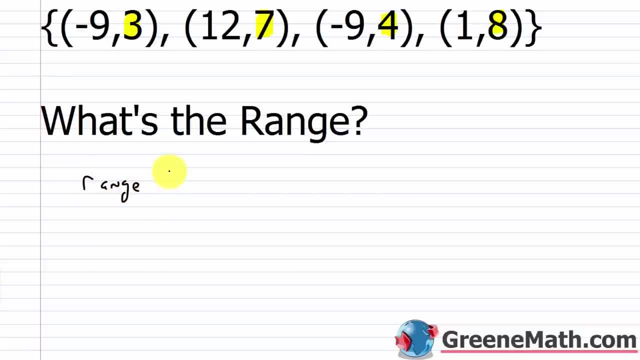 we're going to stop there because this says negative 9 compared to what's separate we're going to take negative 9 comma and subtract negative 9 negit gut nine and then we've gotOH all right now looking at the same relation we want to know 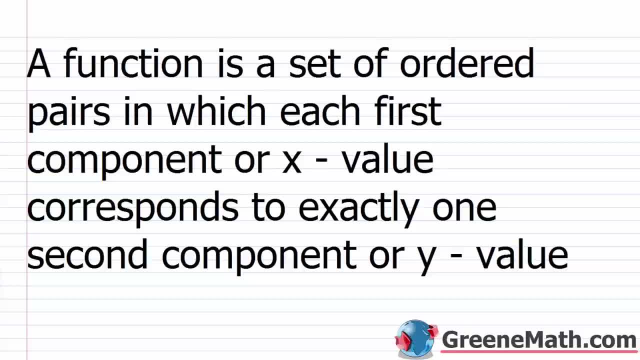 what's the range so the range again is the set of all second components so Y values so 3 7 4 and 8 so that's your range and again seven four and eight all right so now that we've gotten some of the basic kind of vocabulary out 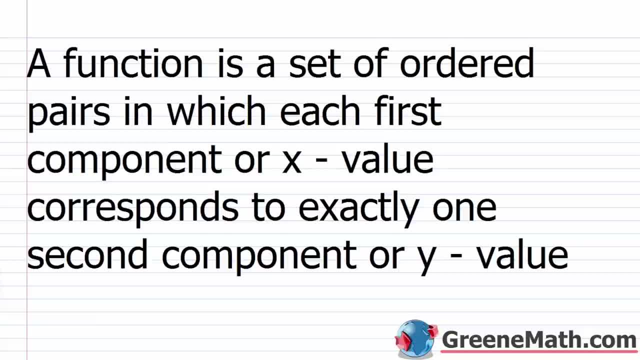 of the way let's start going a little deeper and talking about functions so a function is a set of ordered pairs in which each first component each first component or again that's the x value corresponds to exactly one second component or y value a lot of times you're going 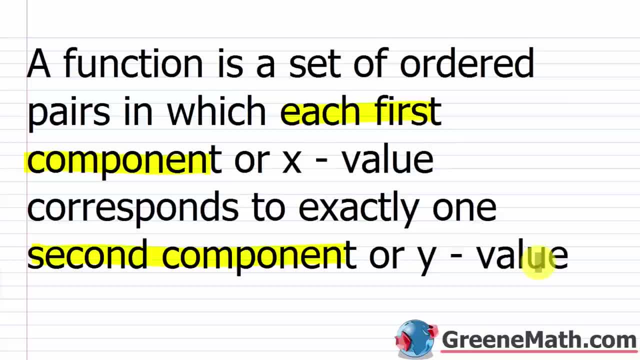 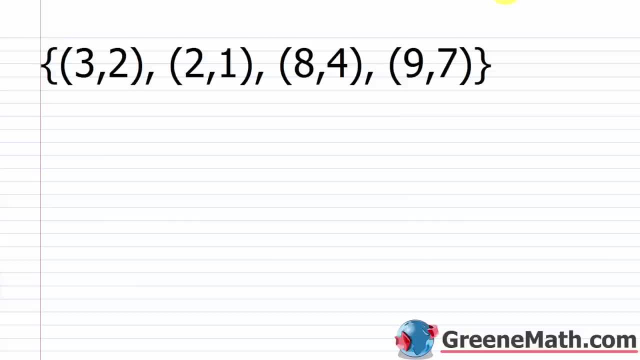 to hear for each x there can be only one y now in order to understand that let's take a look at this relation here so in this relation we have the ordered pair three comma two two comma one 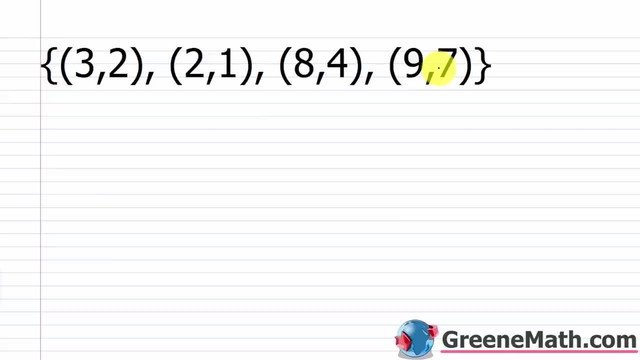 eight comma four and nine comma seven so in other words this is going to be a function and so not every relation is a function but all functions are relations you're going to hear that in your lecture from your teacher or maybe your tutor will say it or maybe you just hear me say it but again all functions are relations 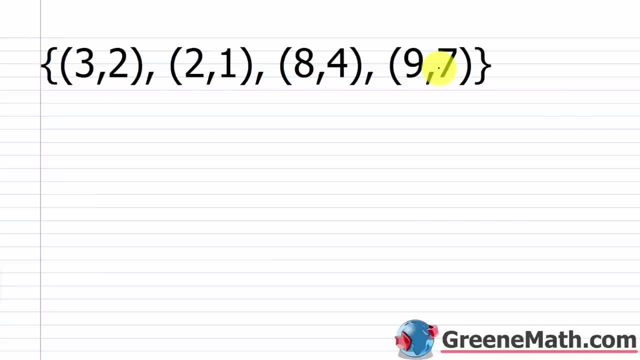 but not all relations are functions so if i look at each ordered pair here this three corresponds 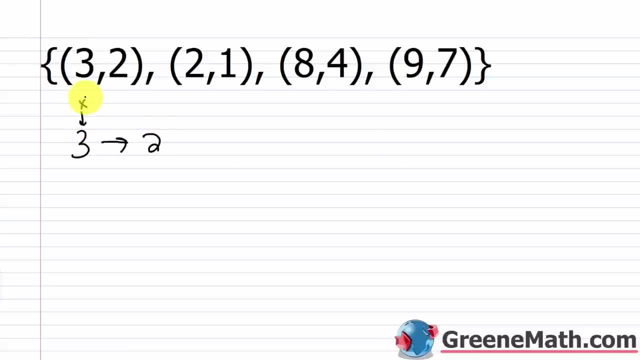 to two so in other words i have an x value that's three i have a y value that's two here i have an x value of two it corresponds to a y value of one here i have an x value of eight it corresponds to a y value of four here i have an x value of nine it corresponds to a y value of seven this is a function because for each x that i have it corresponds to exactly one y value okay and i know that doesn't really make a lot of sense when you first hear it or see it but let me show you an example of something that's not a function so maybe you'll see it that way so this is an example of a relation that is not a function so you've got a set of ordered pairs but the problem is okay your order appears you have seven comma negative four negative one comma five seven comma three and two comma negative eight so if you think about your x values what do you have you have seven you have negative one you have seven again so remember when we were listing our domain we didn't list it twice so i'm just gonna keep that one seven there and then you have two so what are the y values we have negative four you have five you have three you have negative eight so you can think about this as your x values or again your domain right your list of first components you think about this as your y values or again your range your list of second components now for each x there can be only one y or there can be an association with one y 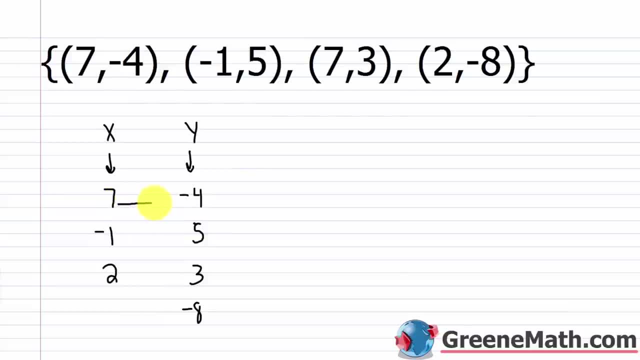 so seven is corresponding to negative four but over here it corresponds to three that is a huge problem now negative one to five that's fine and two corresponds to negative eight that's fine this is the problem right here this seven and when you have a function you have to be able to say okay for this given x value i know what the y value is going to be so if i have an x value of seven i need to have a clear association that i'm going to have a y value of this and i 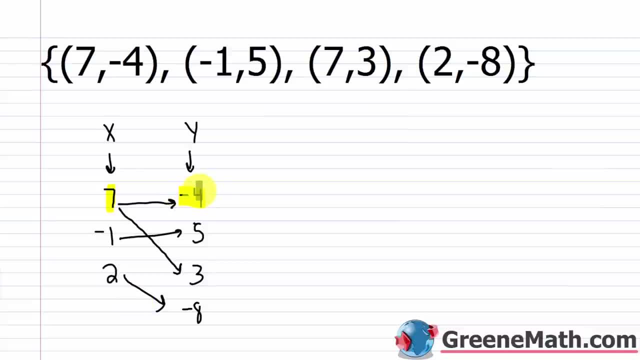 don't here i have two y values i have a y value of and i have a y value of 3. so there's no clear association between this x and the y value of 5 so if you park the y value of 5 well that's fine where's how you TER sihN in one single time that's not going to change nothing is going to change X value and one Y value. It's linked to two different ones, right? So that's a huge problem 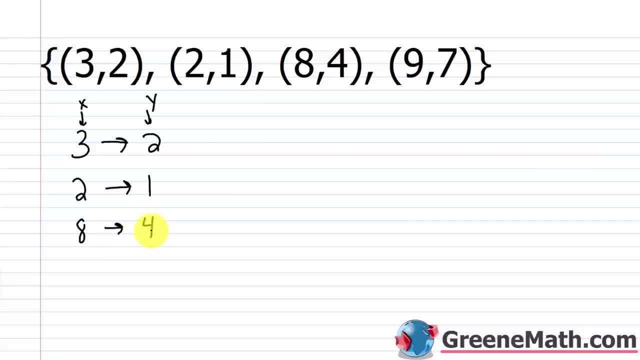 Here I have an x value of eight. it corresponds to a y value of four. Here I have an x value of nine: it corresponds to a y value of seven. This is a function, because for each x that I have, it corresponds to exactly one y value. okay. 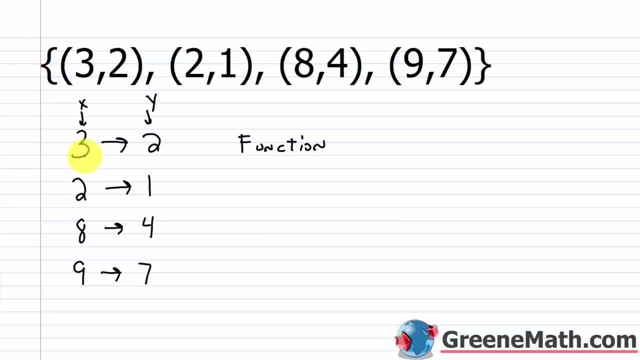 And I know that doesn't really make a lot of sense when you first hear it or see it, but let me show you an example of something that's not a function, So maybe you'll see it that way. So this is an example of a relation that is not a function. 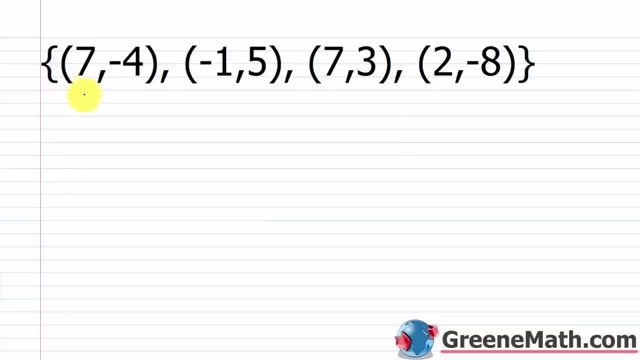 So you've got a set of ordered pairs. but the problem is, okay, your ordered pairs, you have seven comma negative, four negative, one comma five, seven comma three and two comma negative eight. So if you think about your x value, 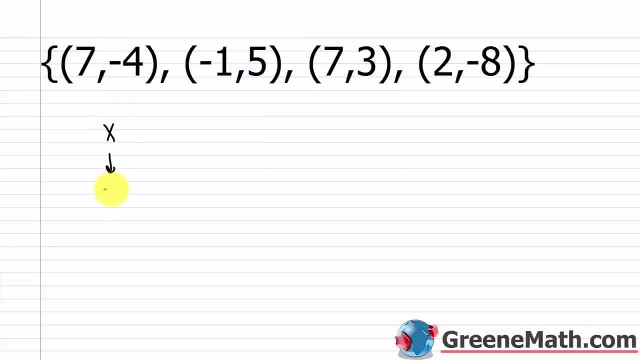 your x values. what do you have? You have seven, you have negative one, you have seven again. So remember when we were listing our domain we didn't list it twice, So I'm just gonna keep that one seven there. and then you have two. 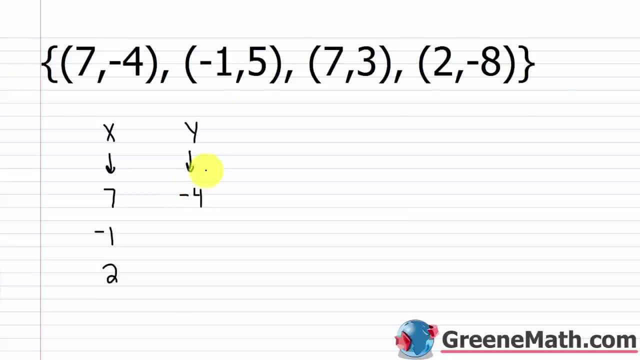 So what are the y values? We have negative four, you have five, you have three and you have negative eight. So you can think about this as your x values or again, your domain right, Your list of first components. 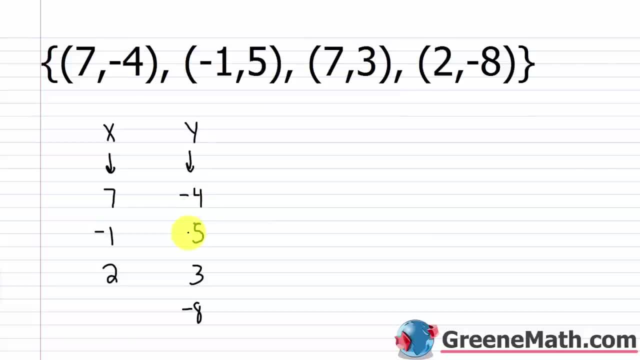 You think about this as your y values, or again your range, your list of second components. Now, for each x there can be only one y or there can be an association with one y. So seven is corresponding to negative four. 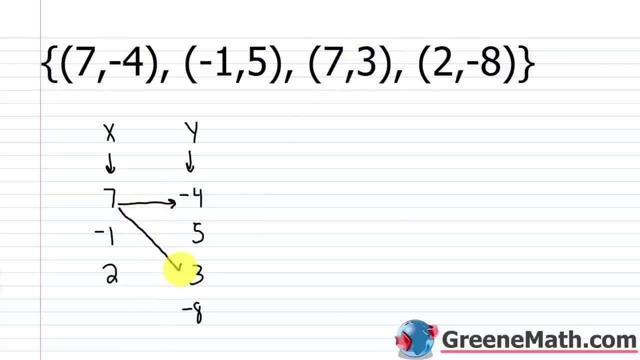 but over here it corresponds to three. That is a huge problem. Now, negative one corresponds to five, that's fine, and two corresponds to negative eight, that's fine. This is the problem right here, this seven, And when you have a function, you have to be able to say: 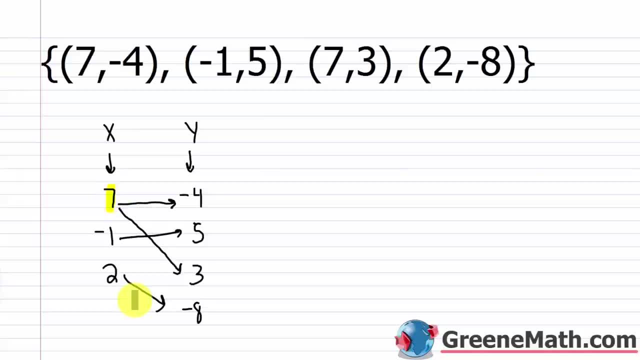 okay for this. given x value, I know what the y value's gonna be. So if I have an x value of seven, I need to have a clear association that I'm gonna have a y value of this And I don't here. 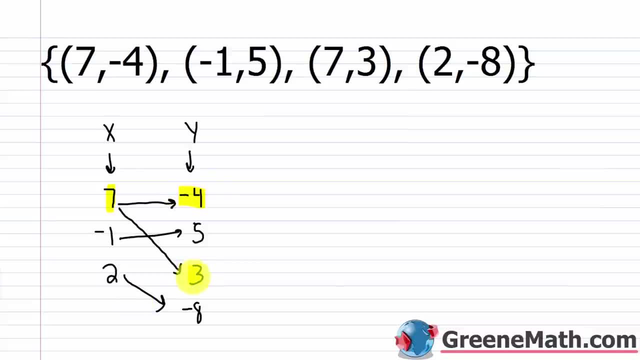 I have two y values, I have a y value of negative four and I have a y value of three. So there's no clear association between this x value and one y value. It's linked to two different ones, right? So that's a huge problem for us. 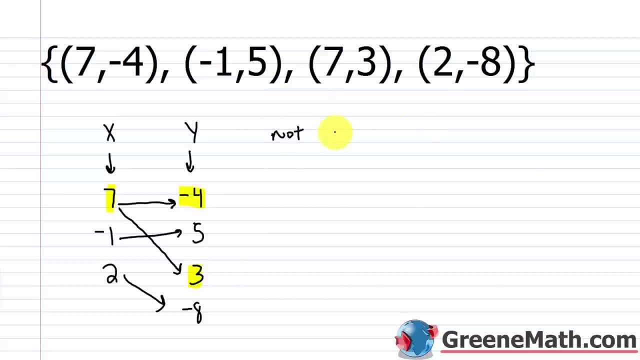 for us. So we're just going to say this is not a function, not a function. And when you first start looking at problems in this section, these are the type of problems you're going to get. They're going to give you a relation, which is basically a set of ordered pairs. And they're going to say, is this a function? Is it not a function? And all you're basically going to do is look for duplicate X values. So if I see an X value here, that's seven, and another X value here, that's 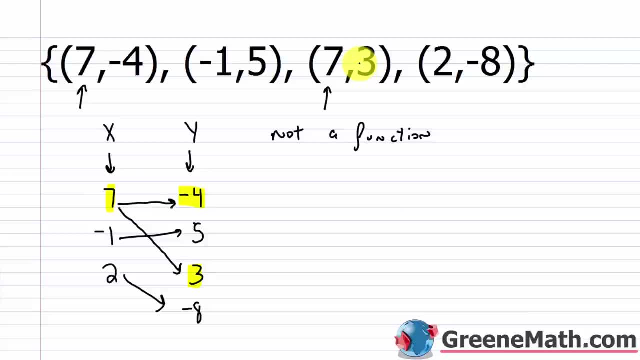 seven, and it's corresponding to two different Y values, I don't have a function. So here's another example we can look at. We have this relation, again, just a set of ordered pairs. We have seven comma negative seven, two comma negative three, six comma five, and negative 12 comma eight. So again, if you see this type of problem, all you're looking for is duplicate X values. I've got a seven, a two, a six, and a negative 12. 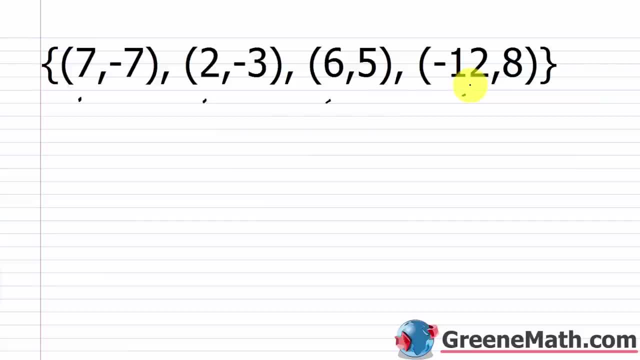 Nothing's duplicated, so this is a function. Because for each X, there's one Y. So every X I have, so in other words, if I said, okay, if I have an X value of seven, what's the Y value? Well, it's negative seven. So if I have an X value of seven, I know that I get a Y value of negative seven. If I have an X value of two, I know I get a Y value of negative three. If I have an X value of six, I know I get a Y value of five. If I have an X value of negative 12, I know I get a Y value of eight. So this is a function. 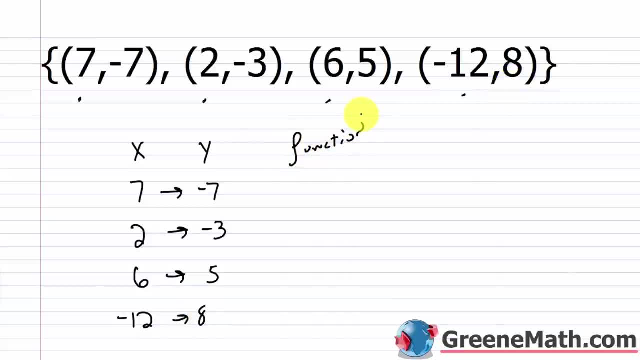 If I was to replace one of these, let's say this wasn't six, let's say this was two. So then in this case, it would not be a function. And why? Well, instead of six being linked to five, I would have two that's linked to negative three and also five. So in other words, if I said, what is the value of Y given that X is two, you really can't give me an answer. You'd have to say, well, it could be negative three or it could be five. So if I said, well, it could be negative three or it could be 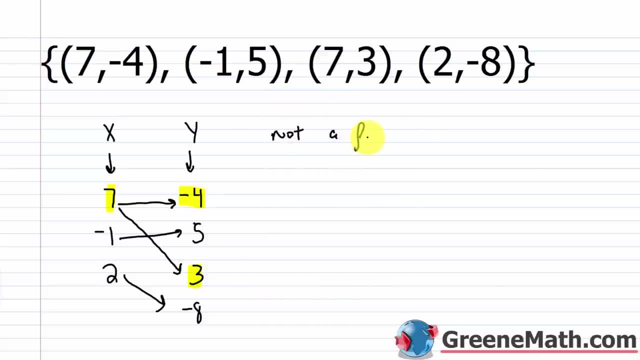 So we're just gonna say this is not a function, Not a function. And when you first start looking at problems in this section, these are the type of problems you're gonna get. They're gonna give you a relation which is basically a set of ordered pairs. 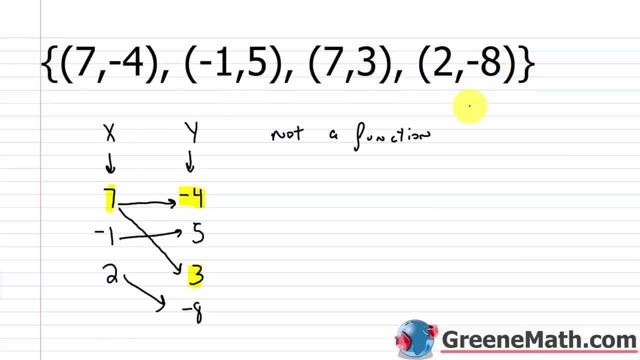 And they're gonna say: is this a function, Is it not a function? And all you're basically gonna do is look for duplicate x values. So if I see an x value here, that's seven, and another x value here, that's seven. 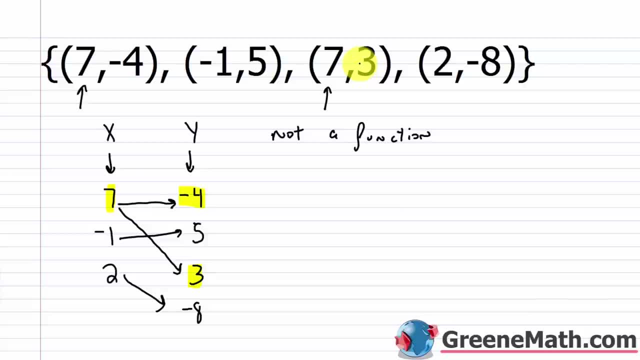 and it's corresponding to two different y values. I don't have a function, So here's another example we can look at. We have this relation, Again, just a set of ordered pairs. We have seven comma negative seven, two comma negative three. 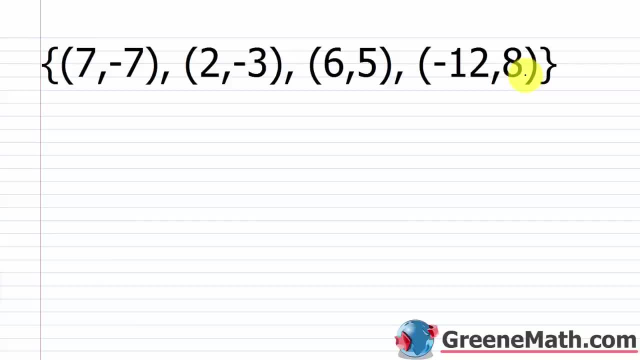 six comma five and negative 12 comma eight. So again, if you see this type of problem, all you're looking for is duplicate x values. I've got a seven, a two, a six and a negative 12. Nothing's duplicated, so this is a function. 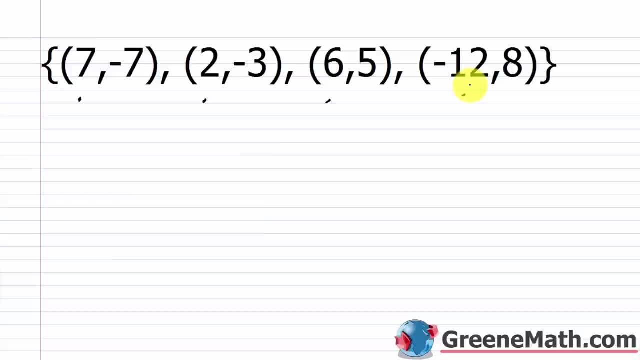 Because for each x there's one y, So every x I have. so, in other words, if I said, okay, if I have an x value of seven, what's the y value? Well, it's negative. It's negative seven. 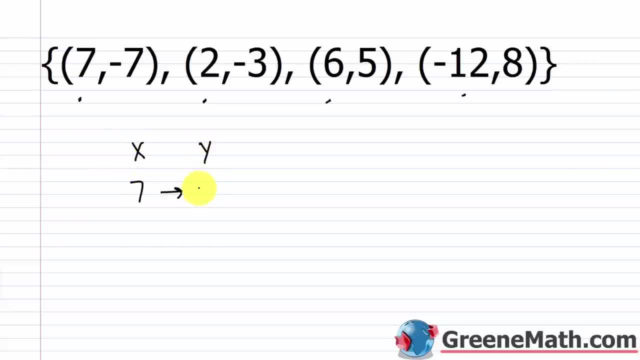 So if I have an x value of seven, I know that I get a y value of negative seven. If I have an x value of two, I know I get a y value of negative three. If I have an x value of six. 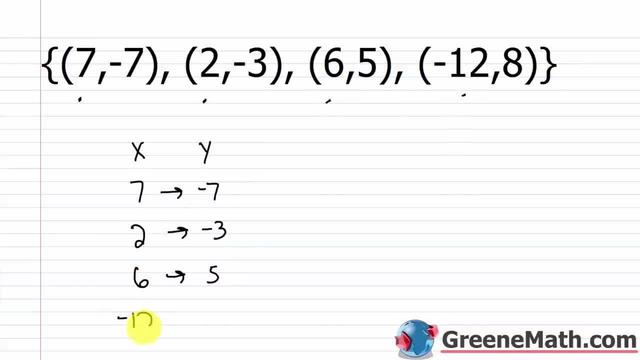 I know I get a y value of five If I have an x value of negative 12,. I know I get a y value of eight. So this is a function. If I was to replace one of these, let's say this wasn't six. 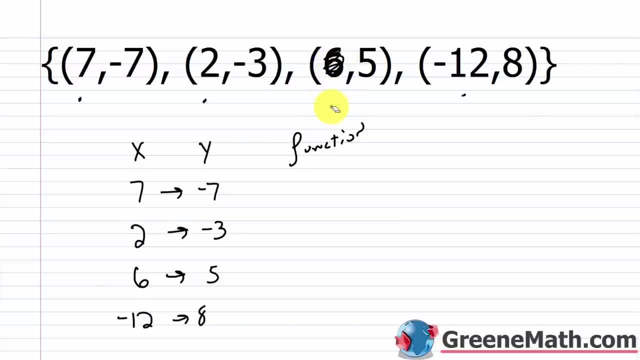 let's say this was two. So then in this case it would not be a function. And why? Well, instead of six, six being linked to five, I would have two, that's linked to negative three and also five. So, in other words, if I said: 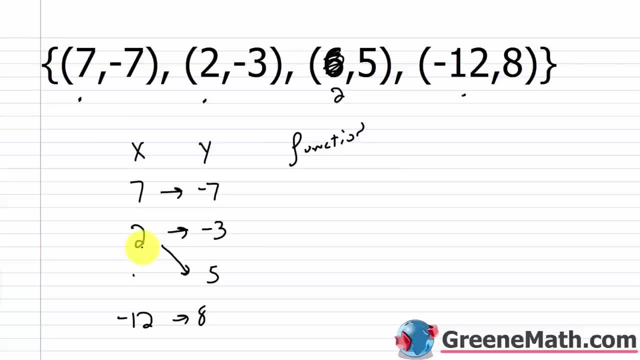 what is the value of y, given that x is two? you really can't give me an answer. You'd have to say: well, it could be negative three or it could be five. I really don't know. And the whole idea behind a function is that 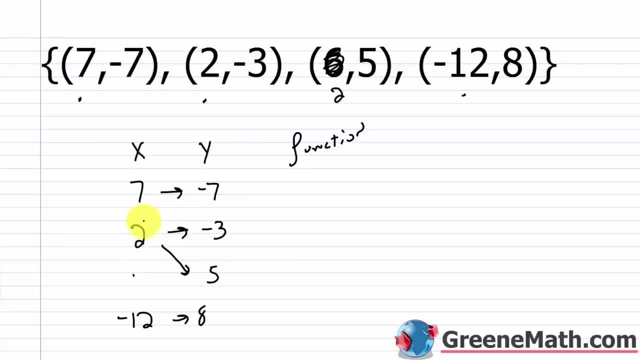 if I give you an x, you can give me a y. So if I say, okay, x is two, you've gotta be able to say, okay, y is negative three. Right, Let me go back to the original example. 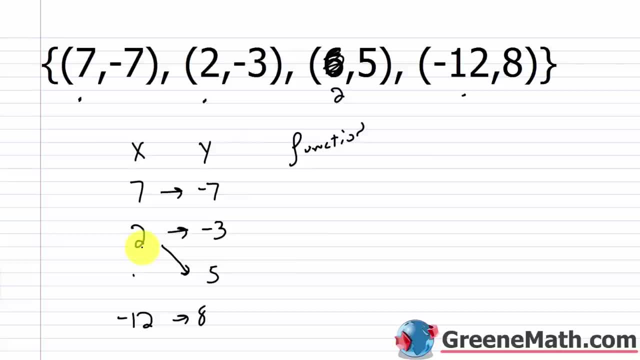 five, I really don't know. And the whole idea behind a function is that if I give you an X, you can give me a Y. So if I say, okay, X is two, you've got to be able to say, okay, Y is negative three. If I go back to the original example, if I give you an X of six, Y is five. So in that case where I replaced this six with a two, two was now linked to two different Y values. And so it wouldn't be a function. But as it's originally written, we have it here where seven is linked to or corresponds to negative seven. Two is linked to 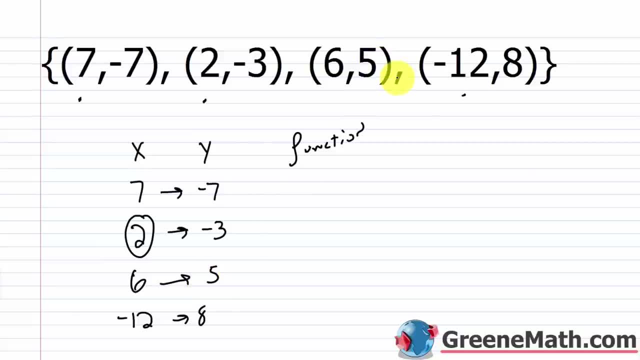 or corresponds to negative three. Six is linked to or corresponds to five. And negative 12 is linked to or corresponds to eight. We do have a function. All right, here's another example. So again, 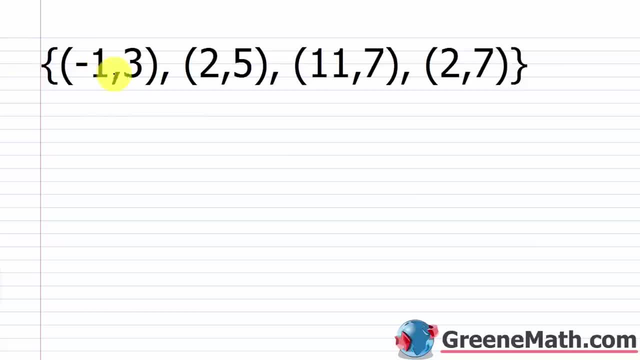 another relation, just a set of ordered pairs. We have negative one comma three, two comma five, 11 comma seven, and two comma seven. So right away, you should notice that you have duplicate 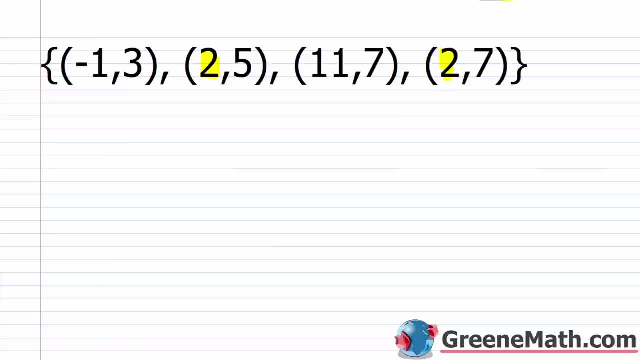 X values. You have a two here and here. That's a problem because, again, if I list this out and I say, okay, my X values and my Y values, so the domain, the set of X values, I'd have negative one, two, and 11 only. For the range 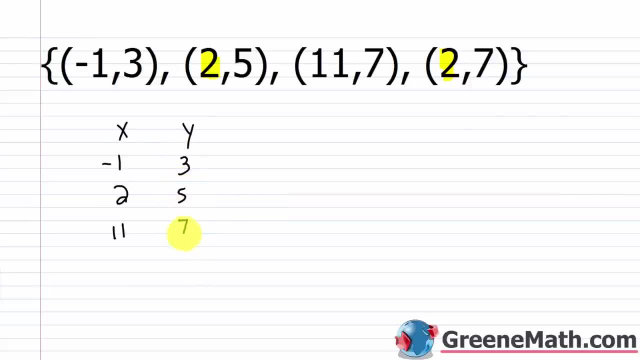 or the Y values, I'd have three, five, seven, and then seven again. Negative one is linked to three. Two is linked to five. Eleven is linked to seven. But then two is also linked to seven. 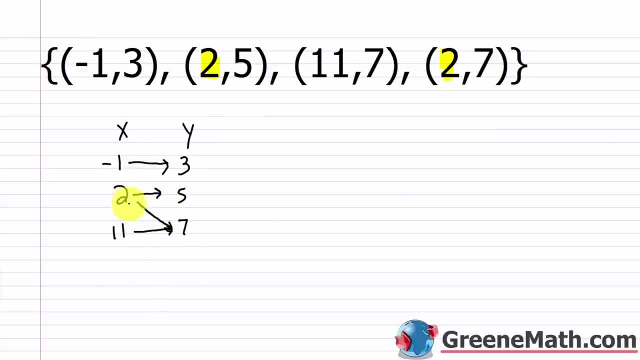 So that's where we have a problem. If I tell you what is the value of Y, given that X is two, you don't know. You'd have to say, well, it could be five or it could be seven. There has to be a crystal clear association. So it has to be, I give you an X and you can 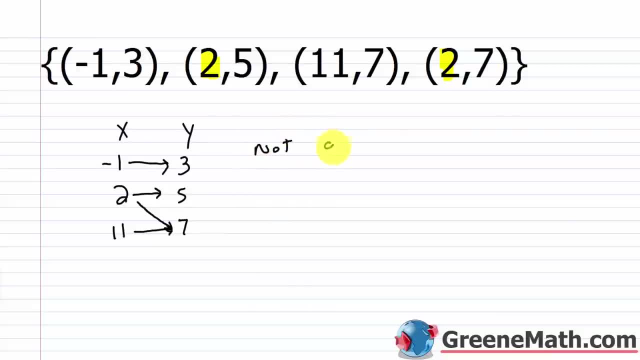 give me a Y. So again, this is not a function. All right, so here's another example. So we have a relation, again, a set of ordered pairs. We have three comma five. 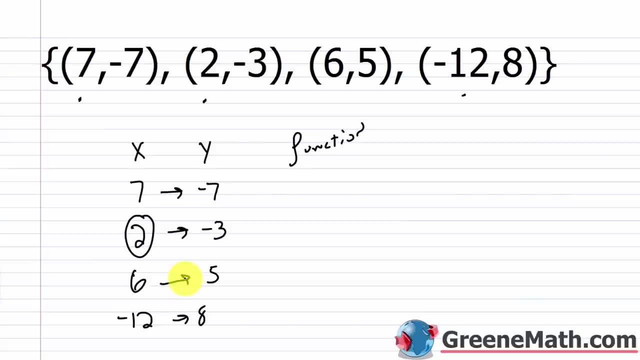 If I give you an x of six, y is five. So in that case, where I replaced this six with a two, two was now linked to two different y values, And so it wouldn't be a function, But as it's originally written, as we have it here, 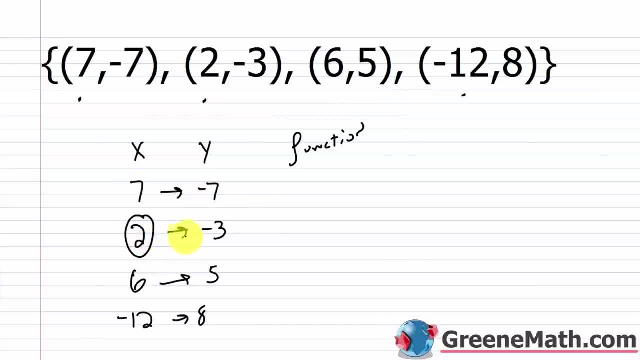 where seven is linked to or corresponds to negative seven, two is linked to or corresponds to negative three, six is linked to or corresponds to five, and negative 12 is linked to or corresponds to eight. we do have a function, All right. here's another example. 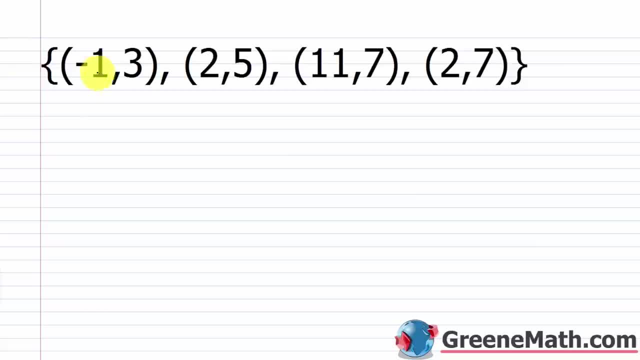 So again, another relation, just a set of ordered pairs. We have negative, one comma three, two comma five, 11 comma seven and two comma seven. So right away you should notice that you have duplicate x values. You have a two here and here. 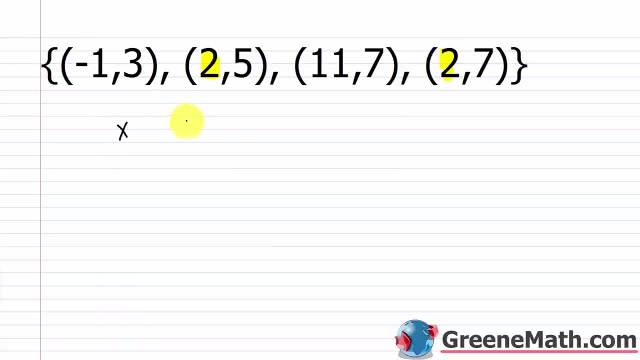 That's a problem because, again, if I list this out and I say, okay, my x values and my y values, so the domain, the set of x values, I'd have negative one, two and 11 only. For the rest of the set of x values, I'd have negative one, two and 11 only. 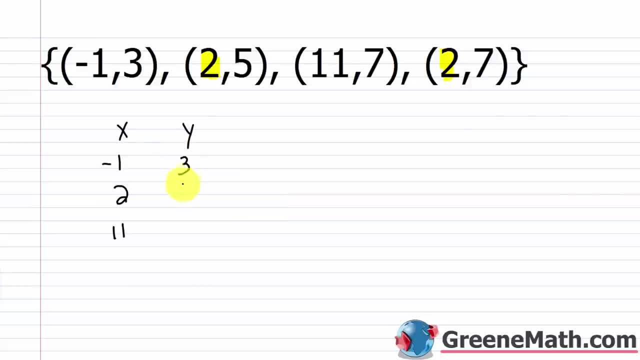 For the rest of the set of x values, I'd have negative one, two and 11. only For the range or the y values, I'd have three, five, seven and then seven again. Negative one is linked to three. 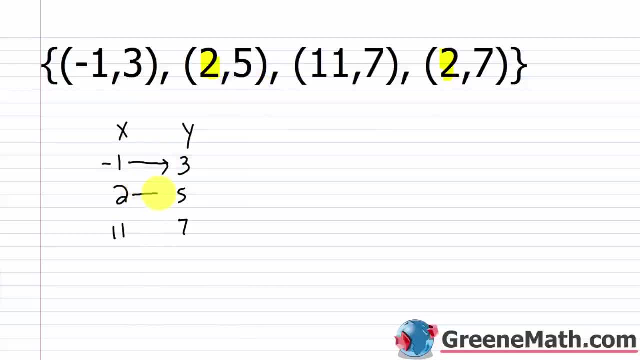 Two is linked to five, Eleven is linked to seven, But then two is also linked to seven. So that's where we have a problem. If I tell you what is the value of y, given that x is two, you don't know. 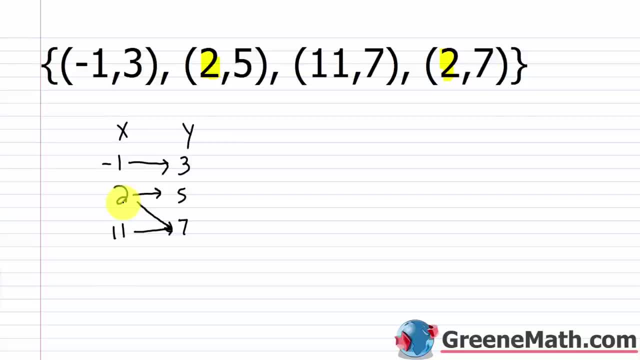 You'd have to say: well, it could be five or it could be seven. There has to be a crystal clear association. So it has to be: I give you an x and you can give me a y. So again, this is not a function. 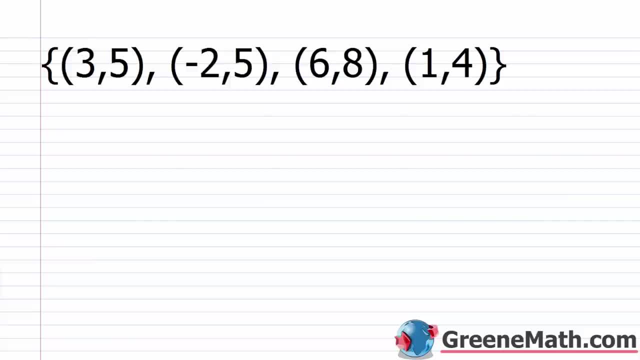 So here's another example. So we have a relation, again, a set of ordered pairs. We have 3 comma 5. We have negative 2 comma 5. We have 6 comma 8. And we have 1 comma 4.. 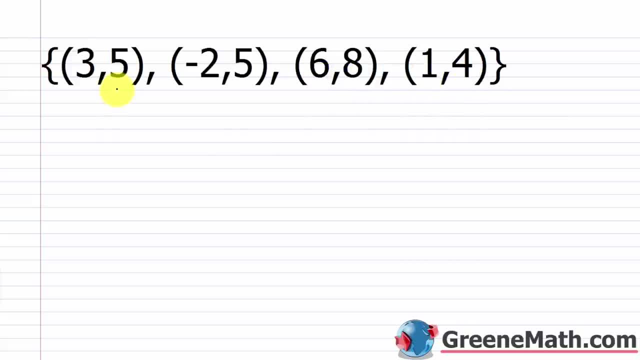 So some of you right away will make the mistake of saying, oh, I have a 5 here and a 5 here, Not a function. You would be wrong. You only need to look for duplicate x values. OK, And I'm going to show you why that's the case in a second. 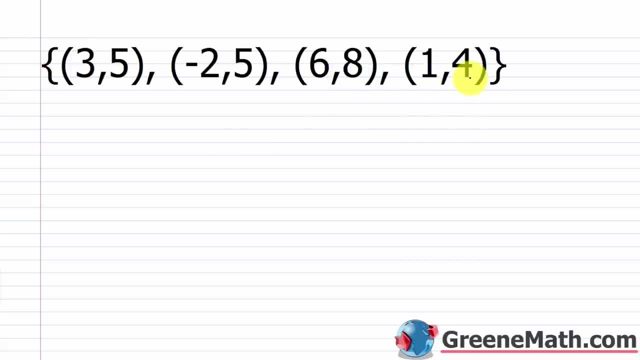 We have negative two comma five. We have six comma eight. And we have one comma four. So some of you right away will make the mistake of saying, oh, I have a five here and a five here, not a function. You would be wrong. You only need to look for duplicate X values. Okay. And I'm going to show you why that's the case in a second. But essentially, again, I have three, 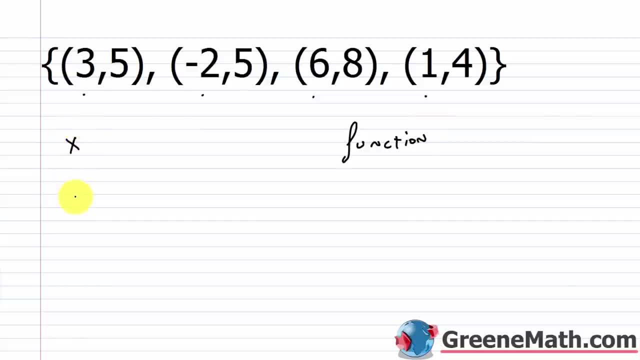 And if you kind of list it out, like, we've been doing. So the X values are the domain. We have three. We have negative two. We have six. And we have one. And then the Y values are the range. We have five. We have five again. We have eight. And we have four. Now, for each X, there can be one Y. So for this X here, three, 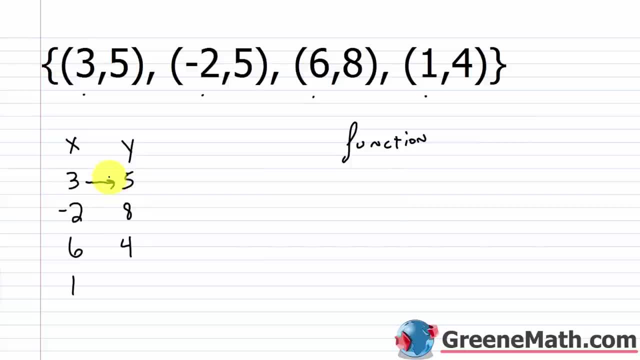 it corresponds to five. So if I say, hey, what is the value of Y in this relation, given that X is three, you can answer five, right? There's no other answer. 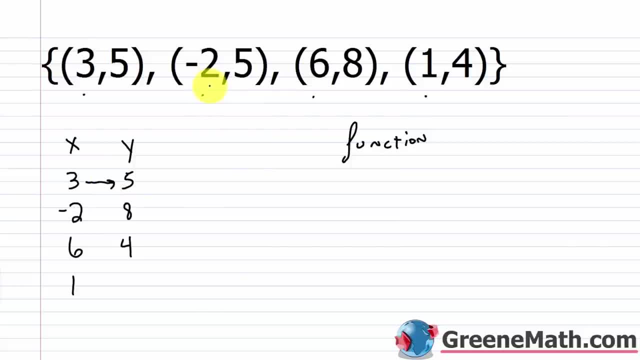 If I say, what is the value of Y if X is negative two, your answer is also five, but that's okay. Two different Xs can be linked to one Y. No problem. Because if you say, hey, 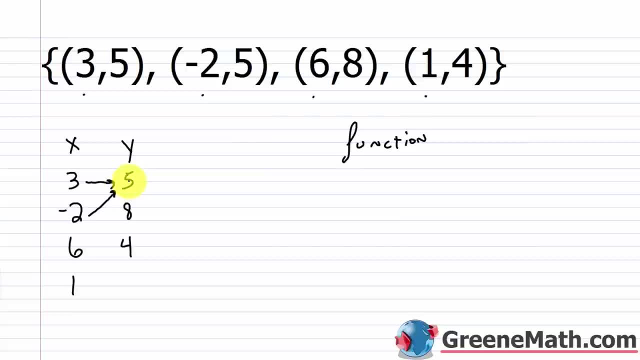 what is the value of Y, given that X is negative two, you have a clear answer. It's five. That's 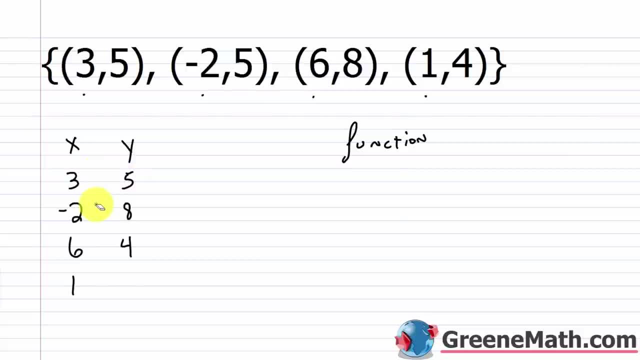 all right. What you can't have, let me erase this real quick. We'll come back to it. Is this going to two different ones? Let's say I had those two ordered pairs in there. I'm going to say, 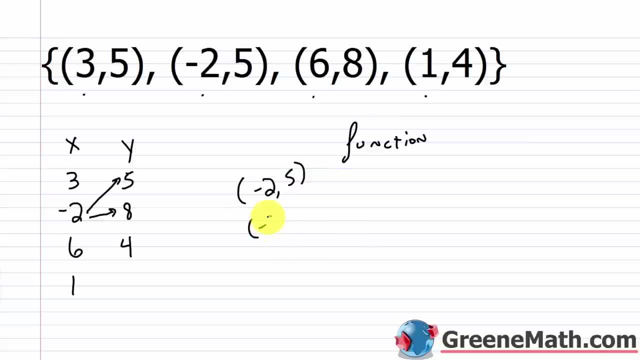 let's say I had something with negative two comma five and negative two comma eight. Well, that's an issue because I'd say, hey, what is the value of Y, given that X is negative two? Well, it could be five, but it also could be eight. There's no clear association between 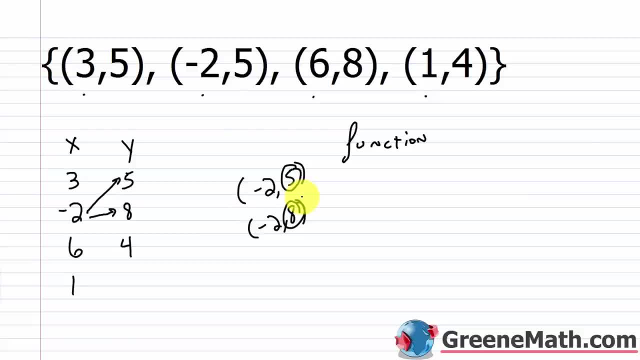 your X value of negative two and some Y value. It's linked up to two different ones. So that's where we have a problem. So again, this is a function because for each X, we have one Y. 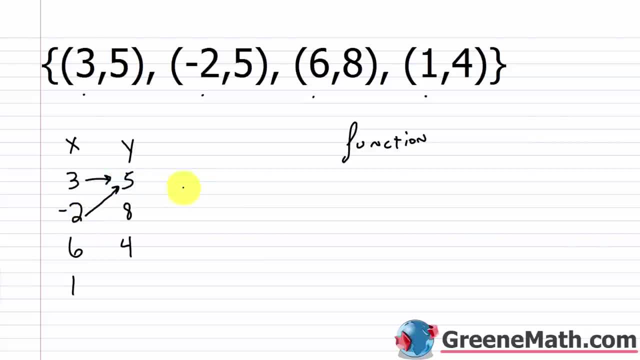 Three. Three corresponds to five. Negative two corresponds to five. Six corresponds to eight. And one 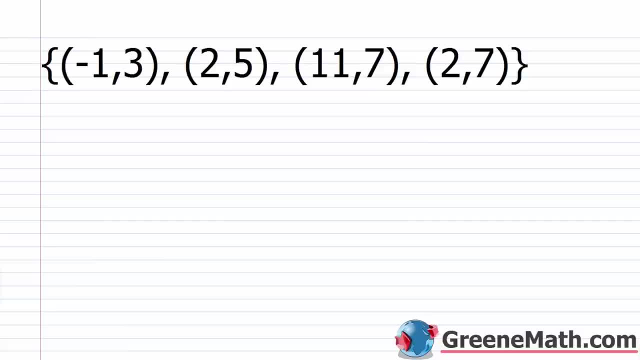 corresponds to four. So I want to kind of revisit one that we know is not a function already. And I want to draw a picture that's probably in your textbook. I'll probably set up something that 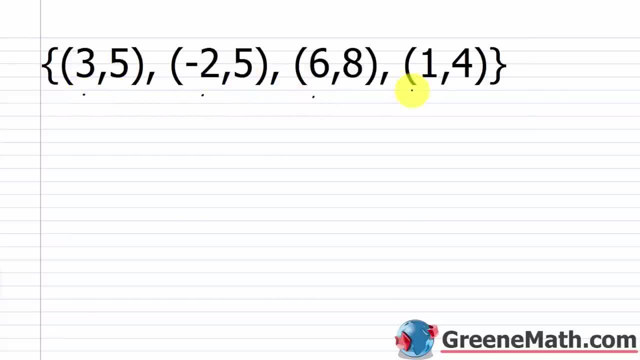 But essentially again, I have 3, negative 2,, 6, and 1.. No duplicate x values. So this is a function And if you kind of list it out like we've been doing, so the x values are the domain. 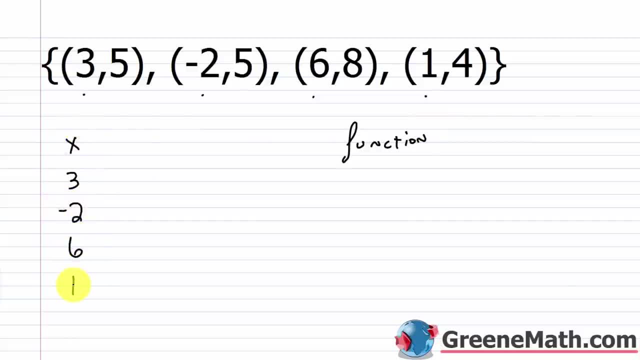 We have 3.. We have negative 2.. We have 6, and we have 1.. And then the y values are the range We have 5.. We have 5, again We have 8.. And we have 4.. 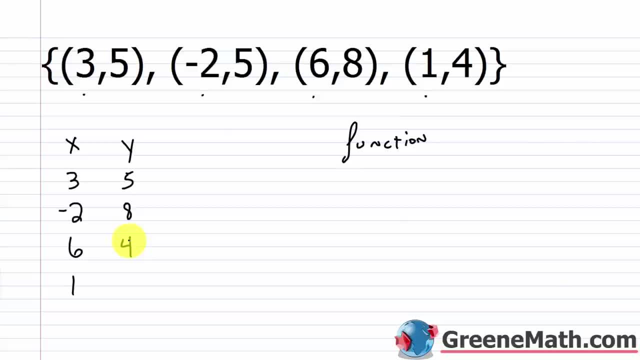 Now, for each x there can be one y. So for this x here, 3,, it corresponds to 5.. So if I say hey, what is the value of y in this relation, given that x is 3?? 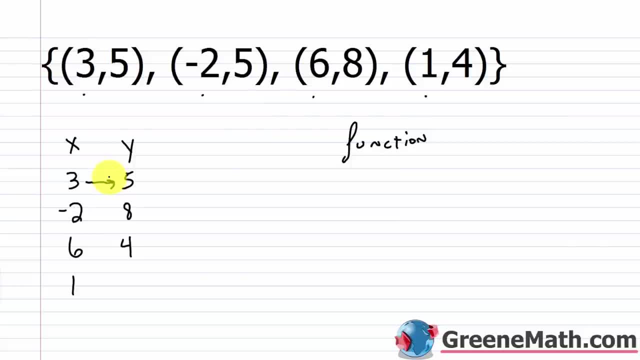 You can answer 5.. There's no other answer. If I say, what is the value of y if x is negative 2?? Your answer is also 5.. But that's OK. Two different x's can be linked to 1y. 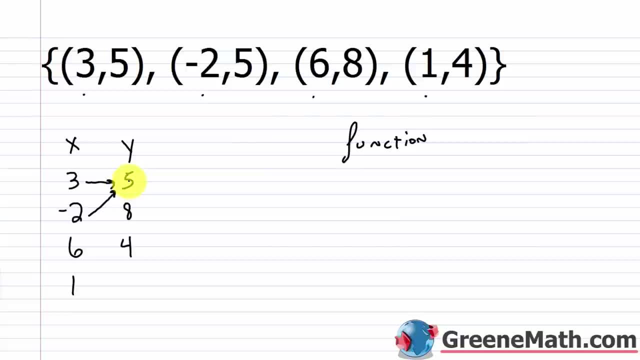 No problem, Because if you say, hey, what is the value of y, given that x is negative 2?, You have a clear answer: It's 5.. That's all right. What you can't have, let me erase this real quick. 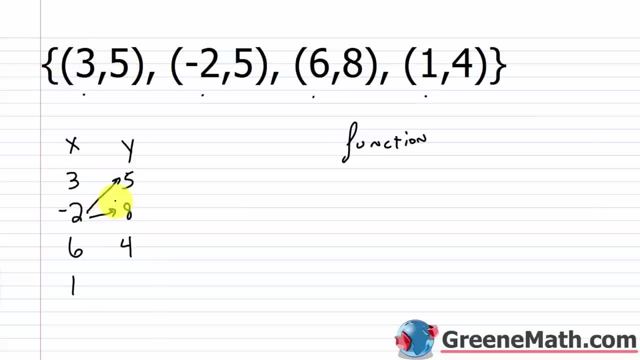 We'll come back to it. Is this going to two different ones? Let's say I had those two ordered pairs in there. Let's say I had something with negative 2, 5 and negative 2, 8.. Well, that's an issue, because I'd say, hey, what is the value? 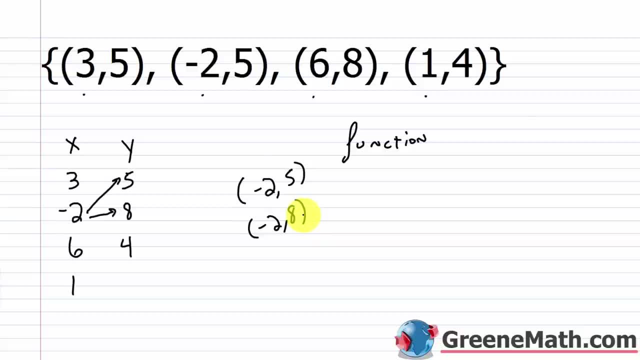 of y, given that x is negative two. Well, it could be five, but it also could be eight. There's no clear association between your x value of negative two and some y value. It's linked up to two different ones. So that's where we have a problem. 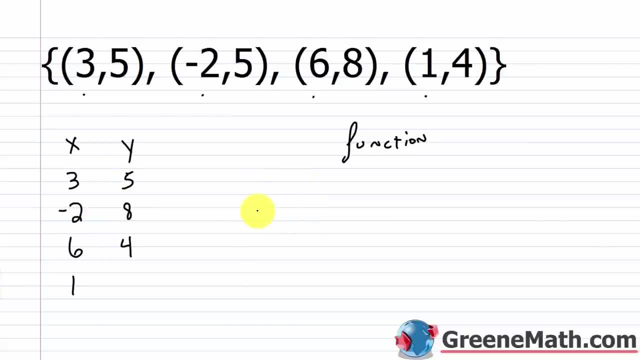 So again, this is a function, because for each x we have one y, Three corresponds to five. negative two corresponds to five, six corresponds to eight and one corresponds to four. So I wanna kinda revisit one that we know is not a function already. 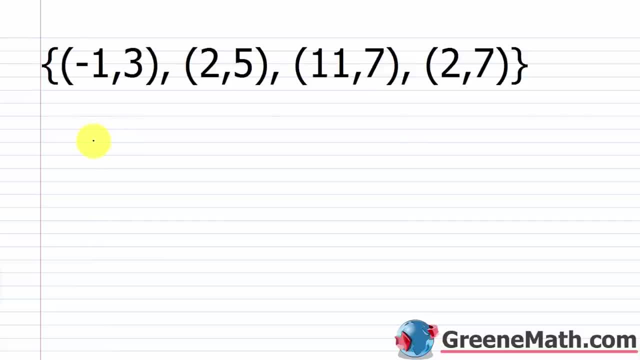 And I wanna draw a picture that's probably in your textbook, or probably set up something that looks like this. So your domain, this is your x values, right, Your set of x values, And we'll draw a little something that looks like this. 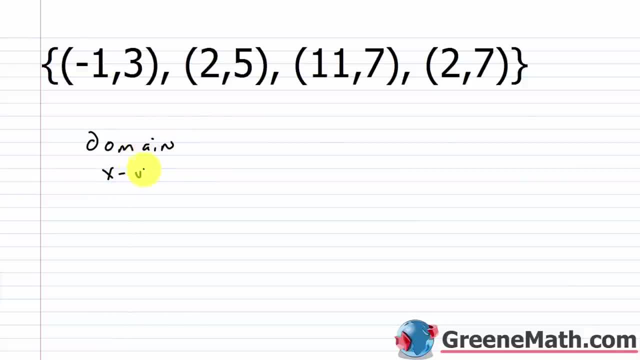 looks like this. So your domain, this is your X values, right? Your set of X values. And we'll draw a little something that looks like this. And we'll list the numbers that are in the domain. So we have negative one. We have two. 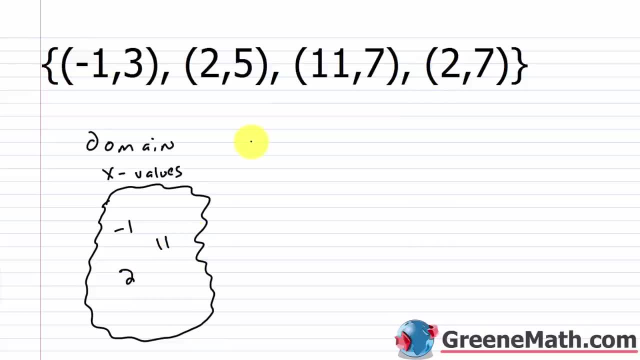 Eleven. And then two again. And then you'll see a picture with the range. Here's the range. Here's the Y values. And in the Y values, or in the land of Y, we have three. We have five. We have 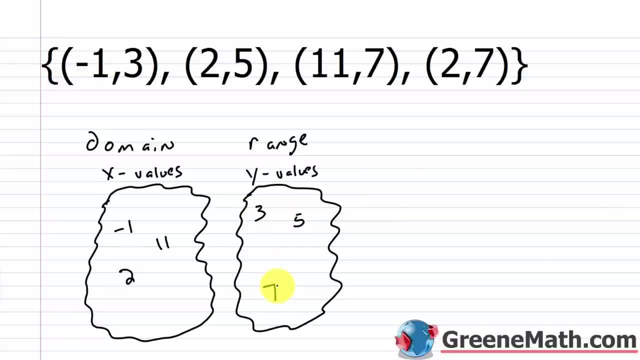 seven. So the problem, or the reason this isn't a function, we have negative one that's linked to three. So if I leave from negative one, I end up at three. If I leave from two, I end up at five. 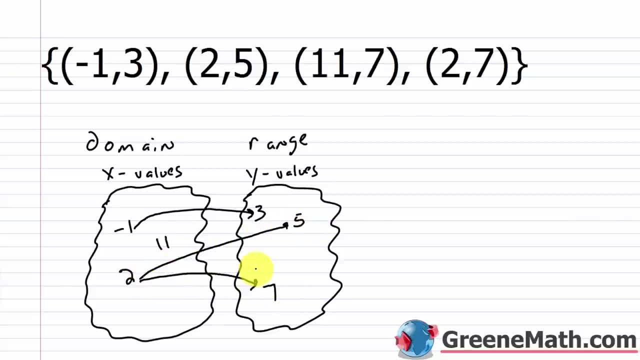 But I also end up at seven. So there's no clear association there. And that's the big problem. I need to know that when I leave from two, I'm going to end up at one location only. If I have a function, I need to have something where I say, okay, X is two, Y is some given value. Here, X is two, and Y could be five, or it could be seven. So again, there's no clear association. And then for 11, that's also linked to seven over here. And here was an example that we did that was a function. So let's do the same. 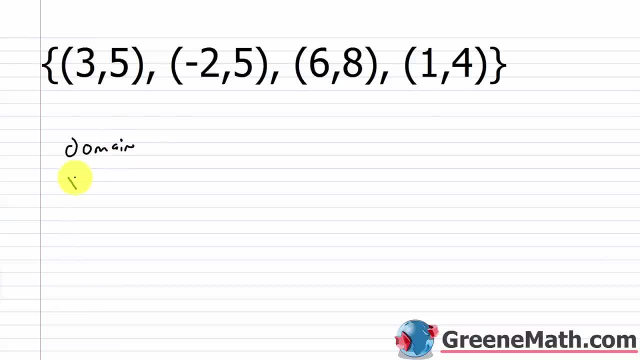 Picture. So we have our domain, or the X values. And let's draw a little picture for those. So we have three, we have negative two, we have six, we have one. And then you have your range, or your set of Y values. So you have five, and that's duplicated. So I just put it once, you have eight, and you have four. So again, for each X, there can be, one Y. So if I leave from three, I know I'm going to five. So there's a clear association. If I leave from negative two, I know I'm going to five. Again, it's okay that two different X's go to one single Y. That's all right. Because in each case, I can say, okay, if I leave from negative two, I know that I'm going to five. If I leave from three, I know I'm going to five. If I leave from six, I know I'm going to eight. If I leave from one, I know I'm going to four. It's only a problem when you leave 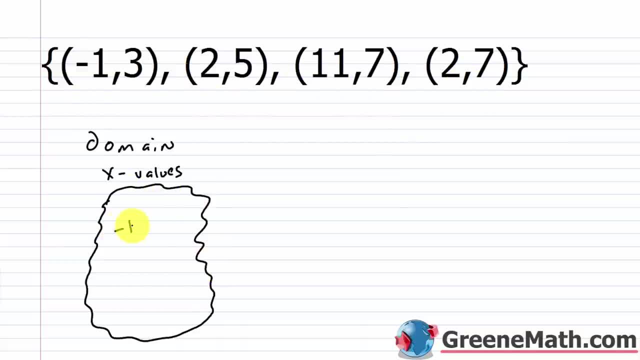 And we'll list the numbers that are in the domain. So we have negative one, we have two, 11, and then two again, And then you'll see a picture with the range. Here's the range. these are the y values. 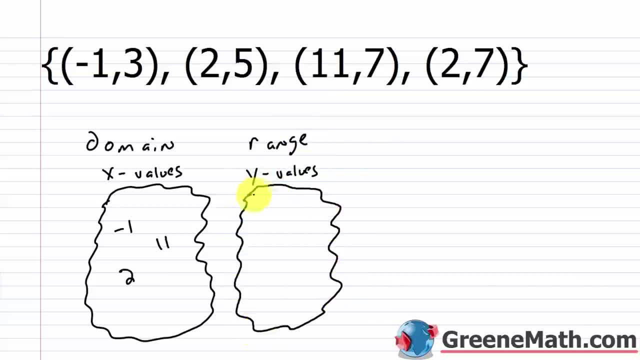 And in the y values or in the land of y, we have three, we have five, we have seven. So the problem or the reason this isn't a function, We have negative one that's linked to three. So if I leave from negative one, I end up at three. 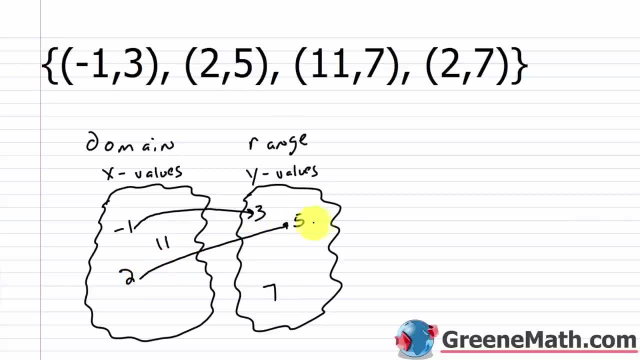 If I leave from two, I end up at five, but I also end up at seven, So there's no clear association there, And that's the big problem. I need to know that when I leave from two, I'm gonna end up at seven. 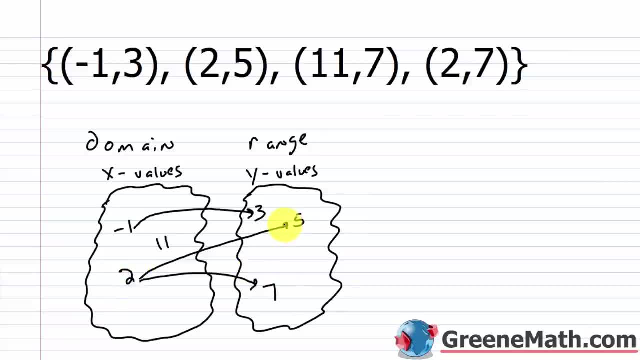 I need to know that when I leave from two end up at one location only If I have a function. I need to have something where I say, okay, x is two, y is some given value Here. x is two and y could be five or it could be seven. So 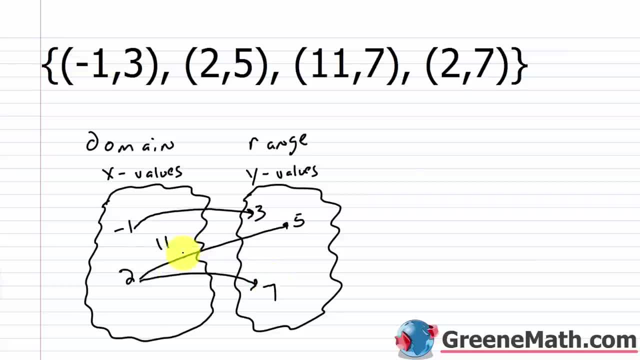 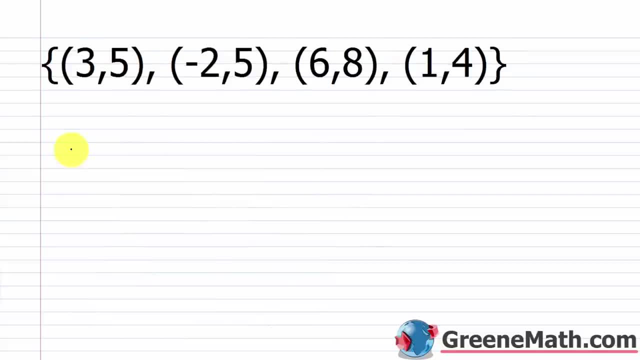 again, there's no clear association. And then for 11, that's also linked to seven over here, And here was an example that we did. that was a function. So let's do the same picture. So we have our domain, or the x values, And let's draw a little picture for those. So we have three. 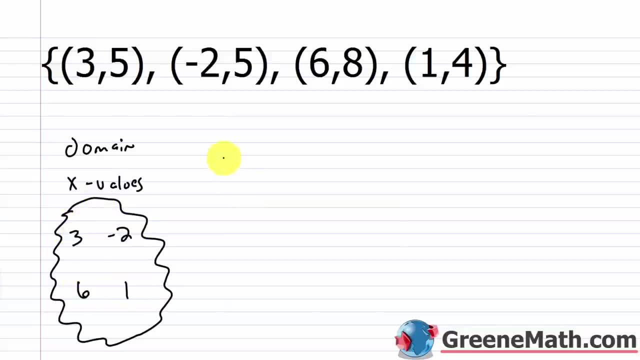 we have negative two, we have six, we have one, and then you have your range or your set of y values. So you have five and that's duplicated. So I just put it once: you have eight and you have four. So again, for each x there can be one y. So 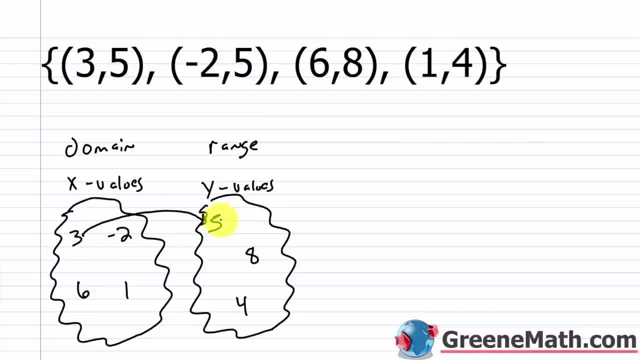 you have five and that's duplicated. So I just put it once: you have eight and you have four. So if I leave from three, I know I'm going to five. So there's a clear association. If I leave from negative two, I know I'm going to five. Again, it's okay that two different x's go to. 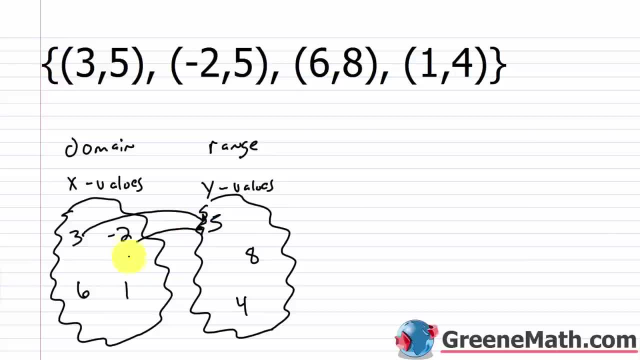 one single y. That's all right, Because in each case I can say: okay, if I leave from negative two, I know that I'm going to five. If I leave from three, I know I'm going to five If I leave. 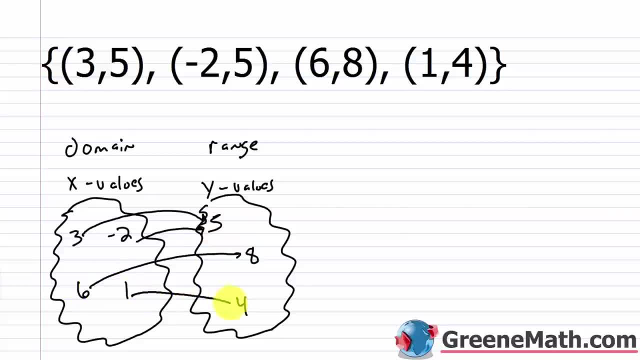 from six, I know I'm going to eight If I leave. from one, I know I'm going to four. It's only a value And you go to multiple y values because then there's no clear association. It's all about. 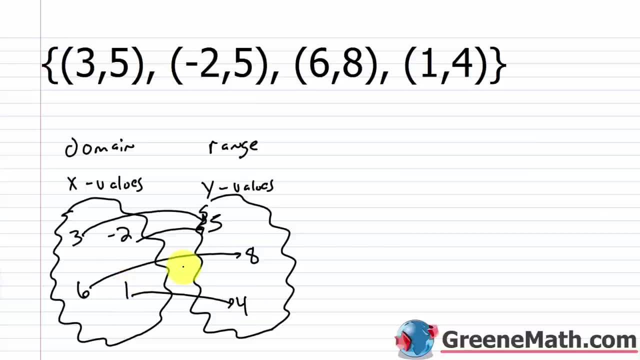 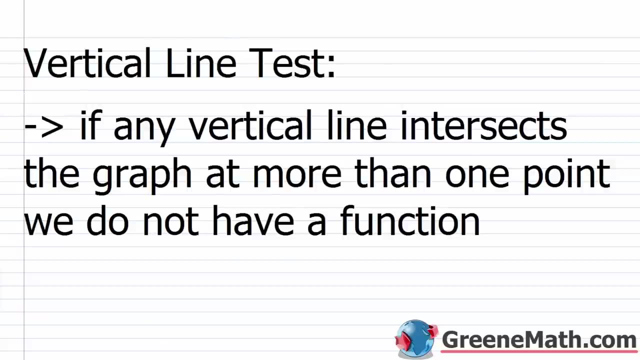 from an X value, and you go to multiple Y values, because then there's no clear association. It's all about give you something for X, you've got to give me one and only one value for Y. Okay, so there's much more to the topic of functions, but kind of in an Algebra 1 course, we're going to just kind of wrap up our lesson and look at something else known as the vertical line test. 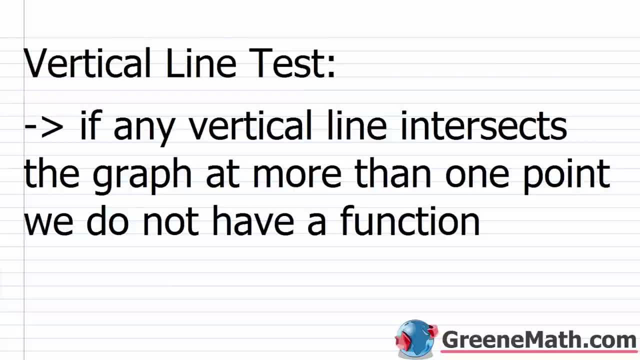 And then we'll kind of leave this topic until we get to Algebra 2, and then we'll get all into the land of functions. 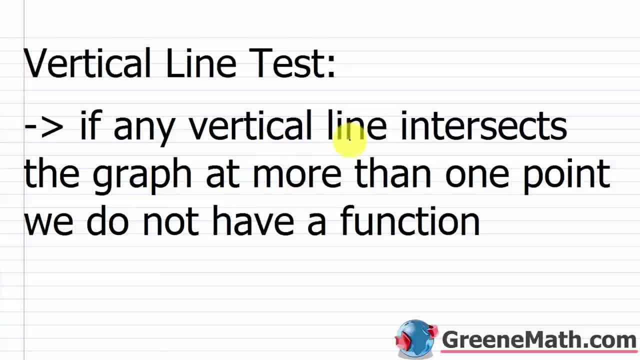 So the vertical line test. If any vertical line intersects the graph at more than one point, we do not have a function. Look at a graph and see why that's the case. So if I look at this coordinate plane, I just have some ordered pasoys. 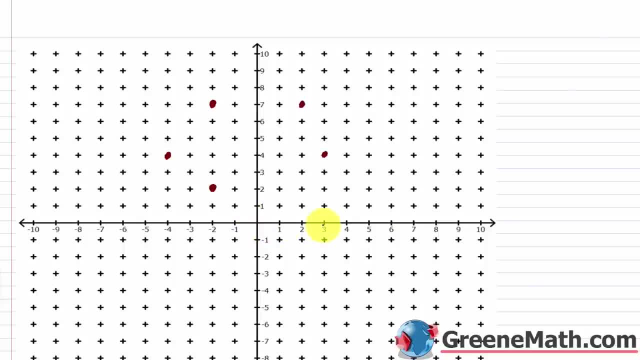 And I want you just to think about that what the ordered pairs for B, so we have three, four, has an order dried Pair, we have two, seven, as an ordered pair, we have negative 22. as an ordered pair. And we have negative 2, 7 as an ordered pair. And we also have negative 4, 4 as an ordered pair. So you can already tell just by looking at the ordered pairs that this wouldn't be a function. Because the x value of negative 2 occurs twice. But you can also determine this graphically by drawing a vertical line. So I'll go through and just make a vertical line really quick. If that vertical line hits the graph in more than one location, you don't have a function. Not a function. 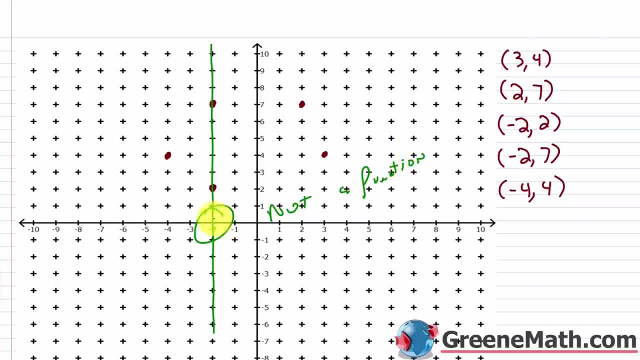 And why is that the case? Well for each x value this x value is negative 2, it can only correspond to one y value. This x value of negative 2 corresponds to a y value of 2. It also corresponds to a y value of 7. 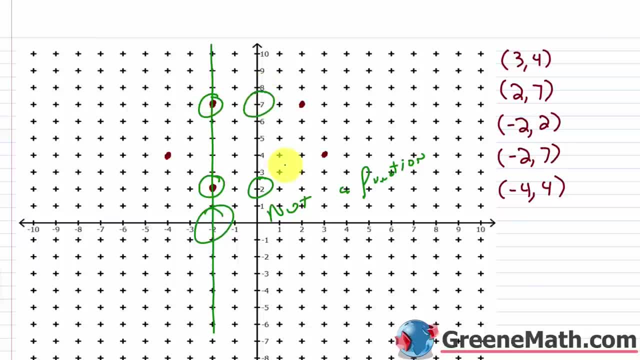 So that's a problem for us. And if you don't have a function you're going to have the scenario where a vertical line is an ordered pair. And if you don't have a function a vertical line will cross at least two ordered pairs 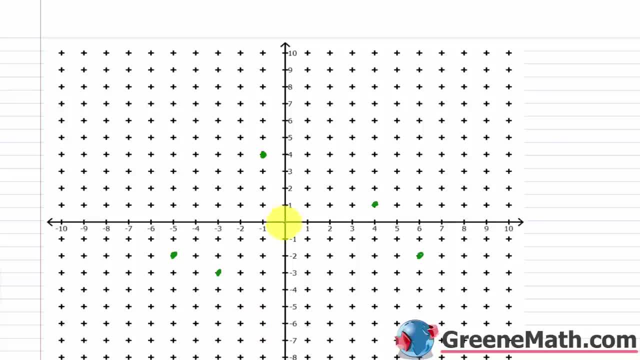 in your relation. So what about something like this where we have the ordered pair negative 5 comma negative 2. Negative 5 comma negative 2. 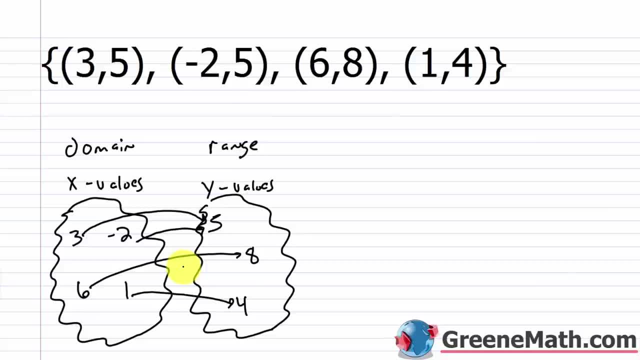 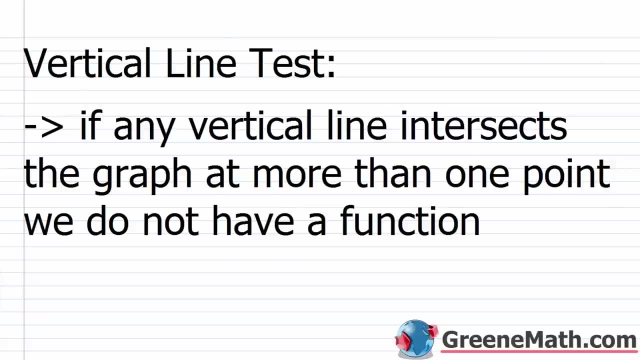 give you something for x, you've got to give me one and only one value for y. Okay, so there's much more to the topic of functions, But kind of in an Algebra 1 course, we're going to just kind of wrap up our lesson and look at something else known as the vertical line test, And then we'll 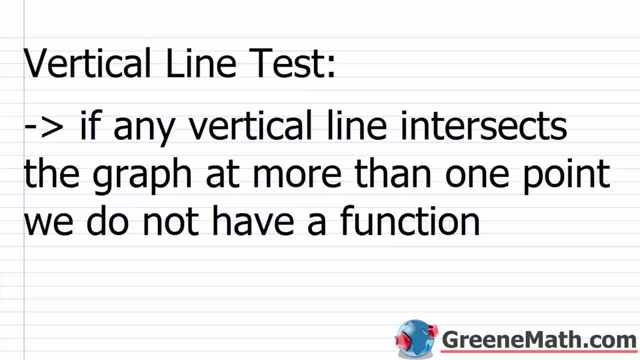 kind of leave this topic until we get to Algebra 2. And then we'll get all into the land of functions. So the vertical line test: if any vertical line intersects the graph at more than one point, we do not have a function. So let's look at a graph and see why that's the case. So if I look 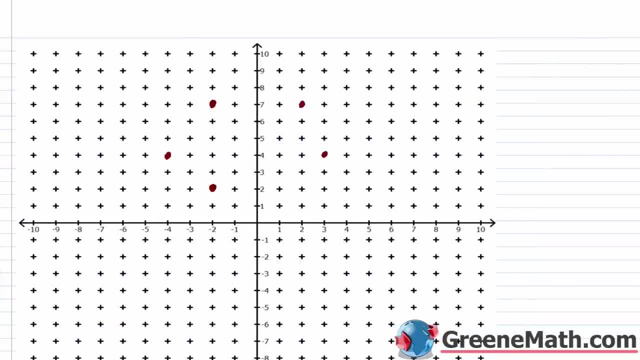 at this coordinate plane. I just have some ordered pairs here And I want you just to think about what the ordered pairs would be. So we have 3, 4 as an ordered pair. We have 2, 7 as an ordered. 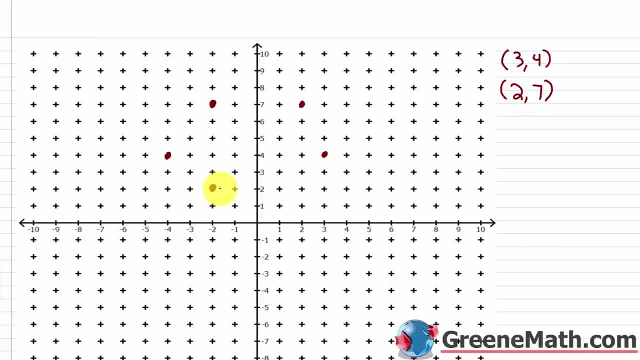 pair. We have negative 2, 2 as an ordered pair, We have negative 2, 2 as an ordered pair, We have negative 2, 2 as an ordered pair And we have negative 2, 7 as an ordered pair, And we also have 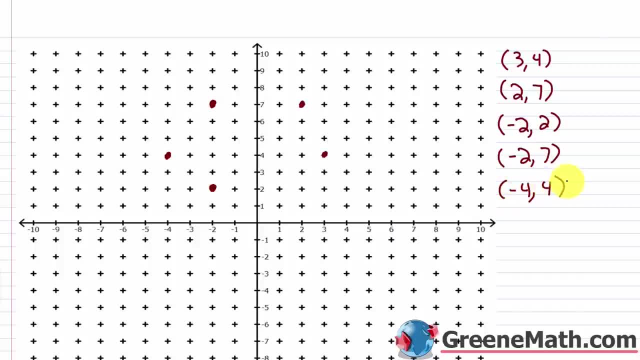 negative 4, 4 as an ordered pair. So you can already tell just by looking at the ordered pairs that this wouldn't be a function right, Because the x value of negative 2 occurs twice. But you can also determine this graphically by drawing a vertical line. So I'll go through and just make a 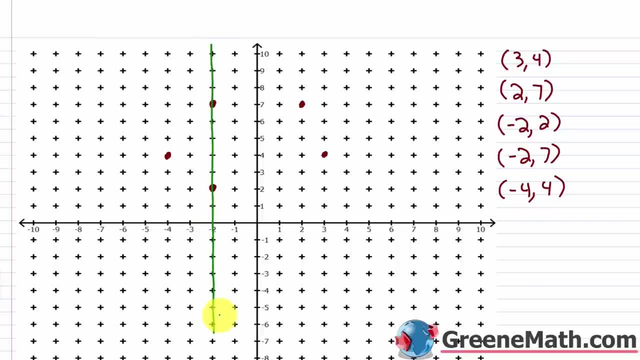 vertical line really quick. If that vertical line hits the graph in more than one point, then we'll be able to see that the vertical line hits the graph in more than one location. You don't have a function, Not a function. And why is that the case? Well, for each x value. okay, this x value is. 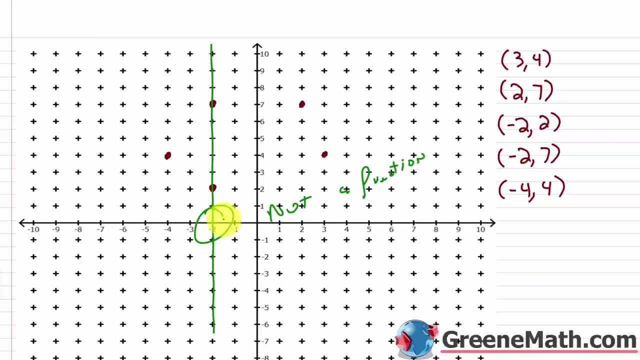 negative 2, it can only correspond to one y value. This x value of negative 2 corresponds to a y value of 2.. It also corresponds to a y value of 7.. So that's a problem for us, And if you don't. 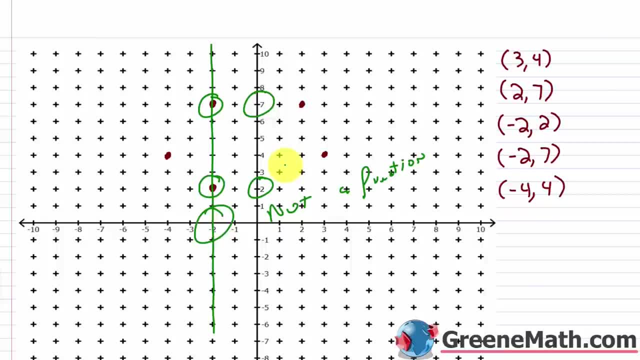 have a function, you're going to have the scenario where a vertical line will cross at least one y value. So if you don't have a function, you're going to have the scenario that the vertical line does not correspond to a y value. Now that's negative 2. You can part. 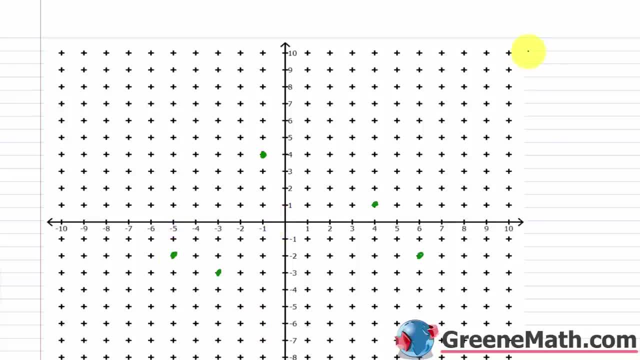 those 2 sides of the equation. After you graduate from college, you have two children. You have two children. You and your child are going to be dating. could you put this line in perspective? I know you have your child back there. go ahead. That works in your theory. So what happens is that the question- oh, you got this number Z all the way through. There's no 2 of these two ordered pairs in your relation. So what about something like this where we have the ordered pairing negative 5 comma-2?? 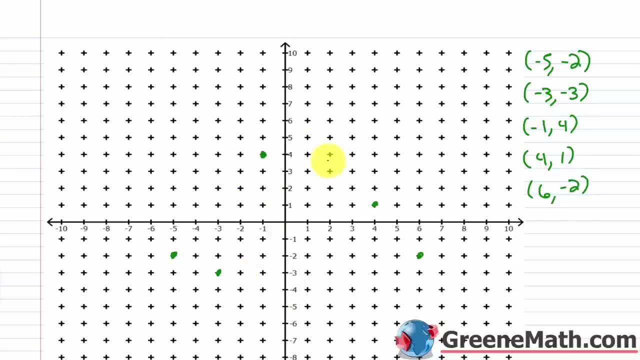 We could see if we made vertical lines going down our coordinate plane, it would never hit in more than one location, meaning it would never cross more than one ordered pair. And the reason for that is: we have a function. We have a function here. 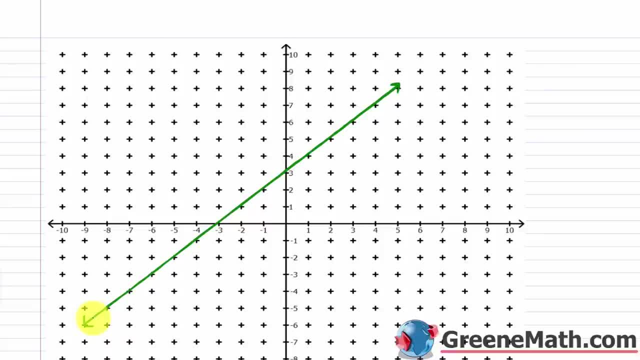 So let's say we came across the graph of a line. Would this be a function? We'll go through and draw some vertical lines and see if it intersects the graph at any place more than once. Well, it doesn't, And I can draw vertical lines all through this thing. 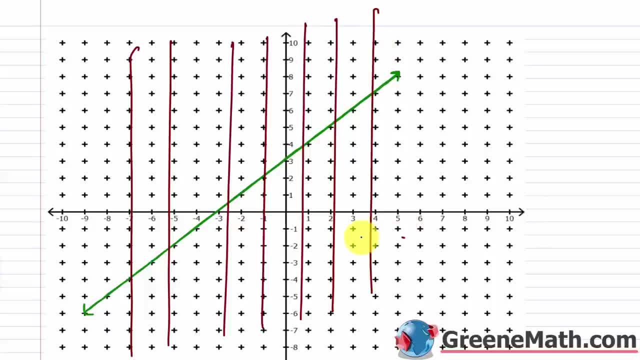 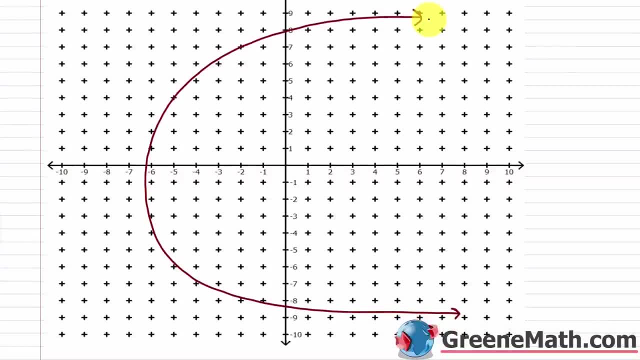 And it's never going to hit more than once. That's because a line is a function, This is a function. What if I saw something like this? Would this be a function? Well, no, it's not. If I look at it, I can tell right away that for each x. 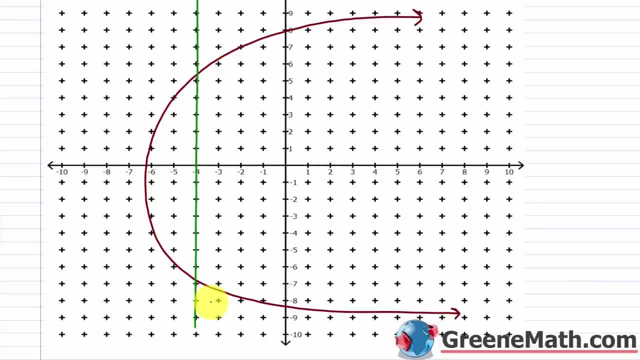 I'm going to have more than one y. If I just draw a line through the x value of negative 4, I can see it. It's going to impact here and also here. So this x value of negative 4 corresponds to two different y values. 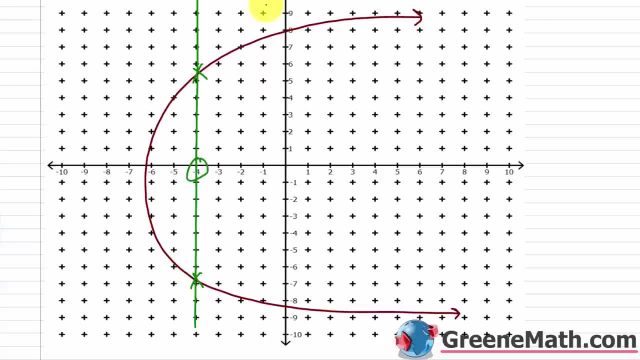 I can go through and make a bunch of different vertical lines. You're going to see, it's going to hit the graph more than once everywhere, Right? So for each x here there's more than one y. So this is not a function. 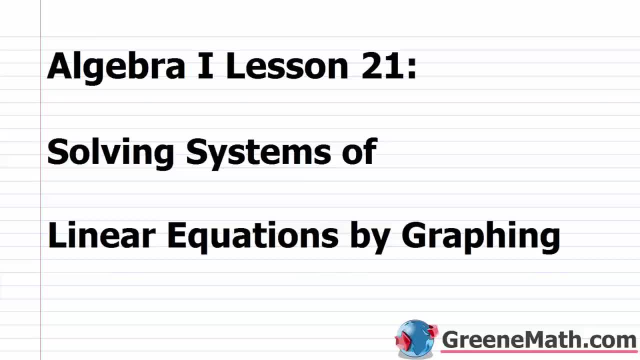 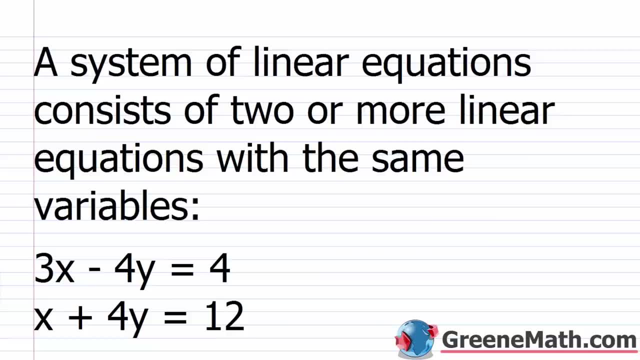 Hello And welcome to Algebra 1,, Lesson 21.. In this video we're going to learn about solving systems of linear equations by graphing. So once we've kind of mastered linear equations in two variables, we move on to kind of the next part of Algebra 1,. 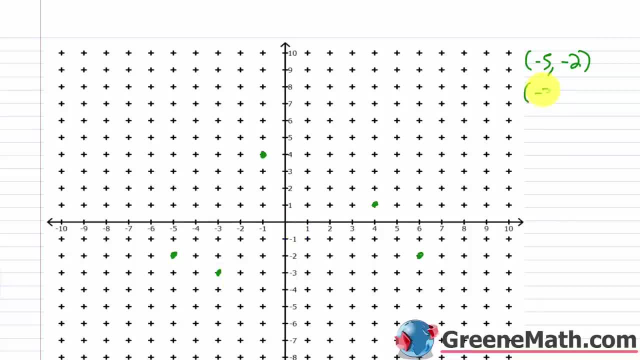 We have the ordered pair negative 3 comma negative 3. We have the ordered pair negative 1 comma 4. We have the ordered pair 4 comma 1. And we have the ordered pair 6 comma negative 2. 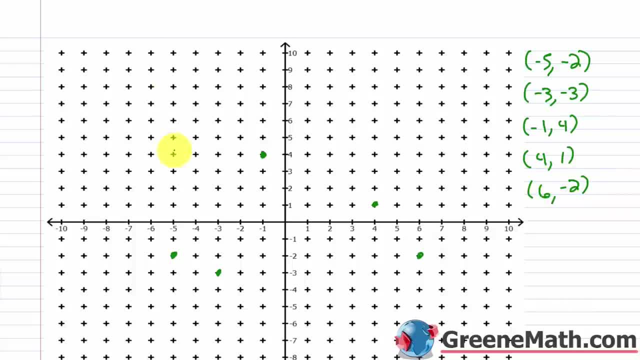 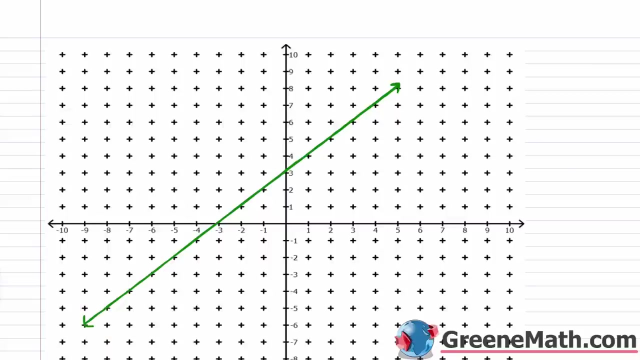 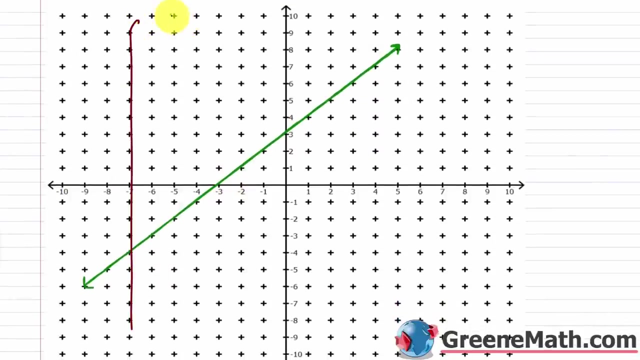 So for this graph, we're going to have a function that's going to correspond to a y value of 7. for this relation here we could see if we made vertical lines going down our coordinate plane it would never hit in more than one location meaning it would never cross more than one ordered pair and the reason for that is we have a function we have a function here so let's say we came across the graph of a line would this be a function we'll go through and draw some vertical lines and see if it intersects the graph at any place more than once well it does and I can draw vertical lines all through this thing and it's never gonna hit more than 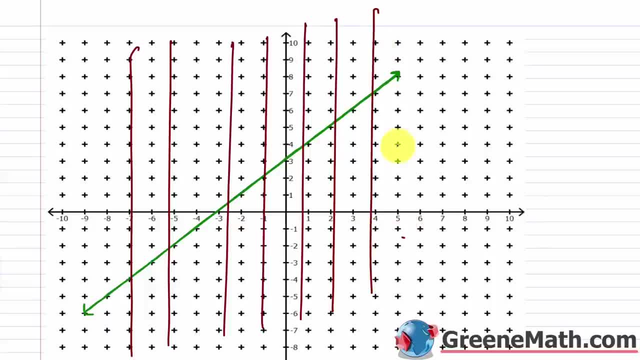 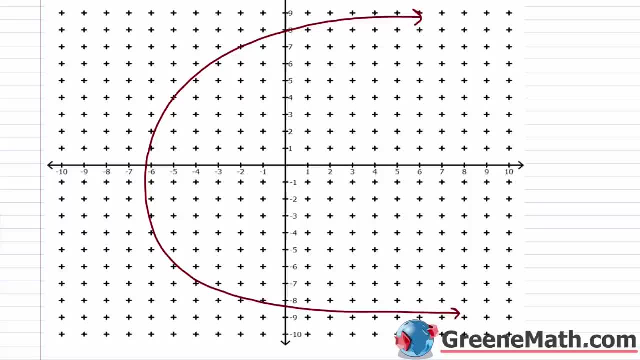 once that's because a line is a function this is a function what if I saw something like this would this be a function well no it's not if I look at it I can tell right away that for each X I'm gonna have more than one Y 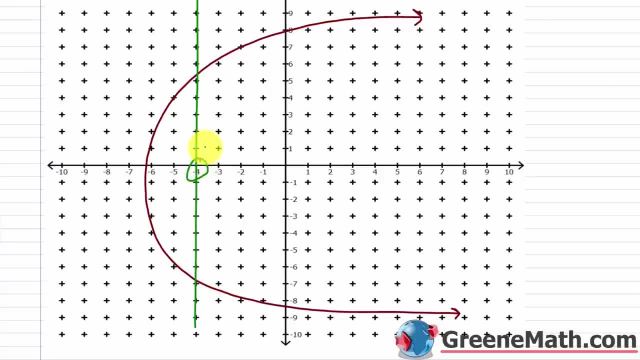 so I just draw a line through the X value of negative four I can see an impact here and also here so this X value of negative four corresponds to two different Y values I can go through and make a bunch of different vertical lines you're gonna see it's going to hit the graph more than once everywhere 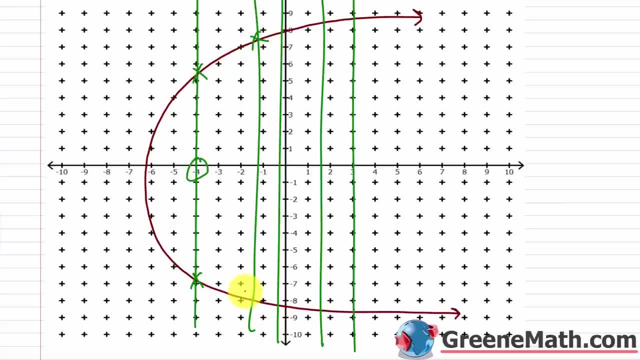 right so for each X here there's more than one Y so this is not good so this is not good 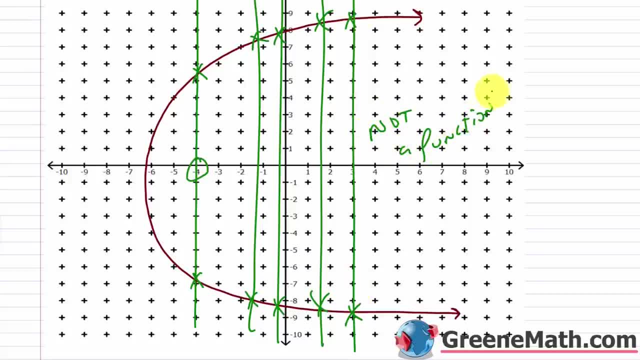 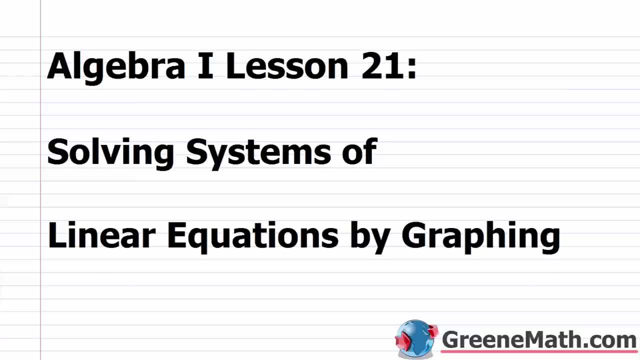 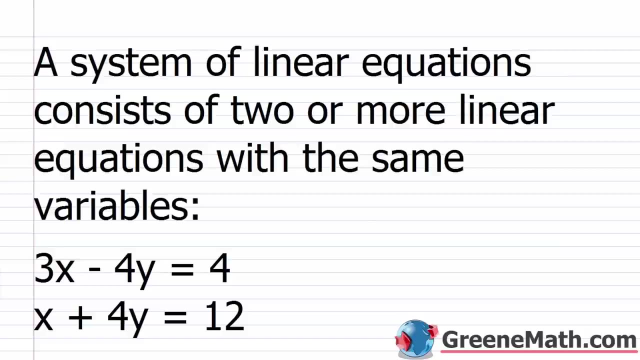 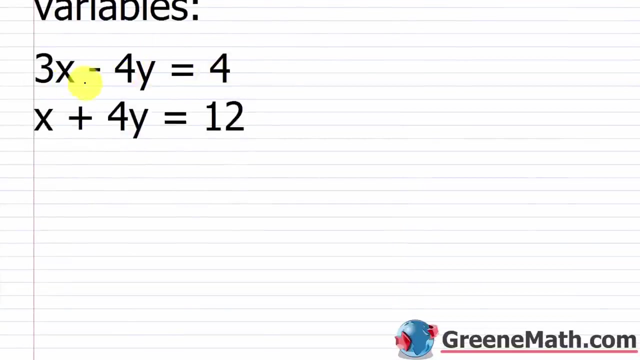 a function. Hello and welcome to Algebra 1 Lesson 21. In this video we're going to learn about solving systems of linear equations by graphing. So once we've kind of mastered linear equations in two variables, we move on to kind of the next part of Algebra 1 where we start talking about systems of linear equations. So a system of linear equations consists of two or more linear equations with the same variables. And mostly in Algebra 1 we're going to have linear systems that just contain two equations. Two equations with two unknowns. So the first example of this that you're going to see, we have 3x minus 4y equals 4. So it's kind of our first equation. And then we have x plus 4y equals 12. So this right here is known as a system of 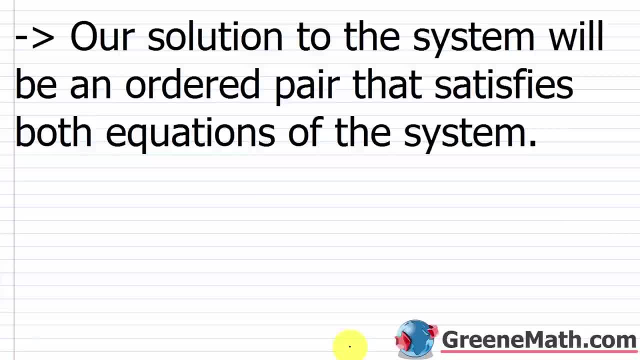 linear equations. So now our solution is going to be slightly different. Because our solution to the system, to the system will be an ordered pair, an ordered pair that satisfies both equations of the system. So if it's a solution to one, but not a solution to the other, it's not a solution to the system. So we're looking for an ordered pair now that's 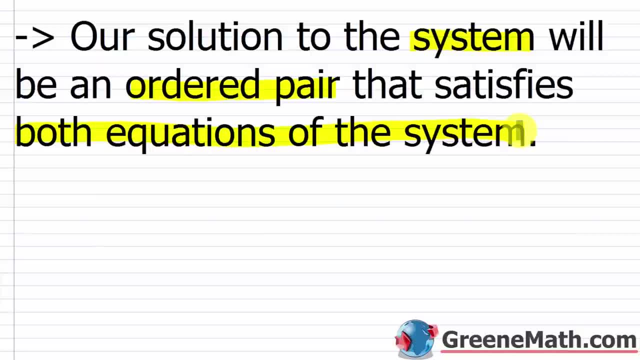 going to satisfy both equations of that system. Or if you have more than two, let's say all three 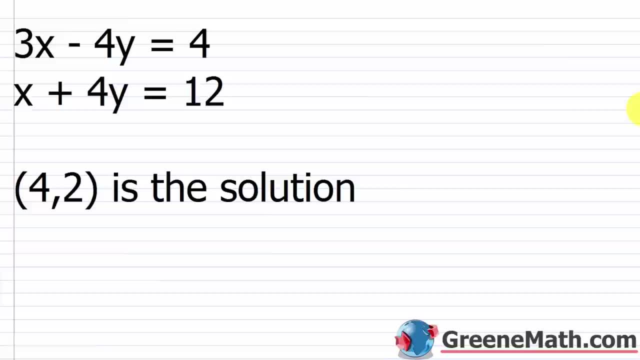 equations simultaneously. Okay, so that's very, very important. All right, so here is an example. 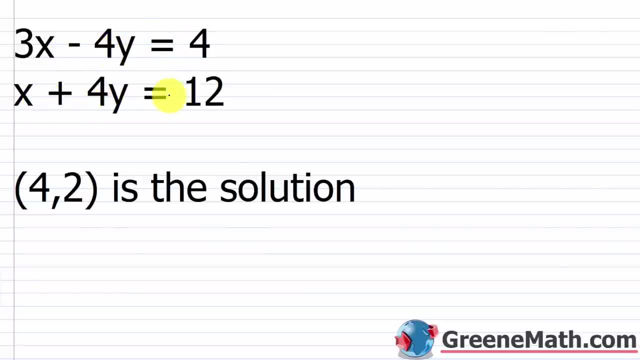 Again, we have 3x minus 4y equals 4, and x plus 4y equals 12. So I'm giving you the solution. The ordered pair 4 comma 2 is the solution. So the way we check this is the same. We plug a 4 in for every x, we plug a 2 in for every y, and we make sure the left and the right side are equal in both equations. So for the first one, we have 3, plug in a 4 for x, 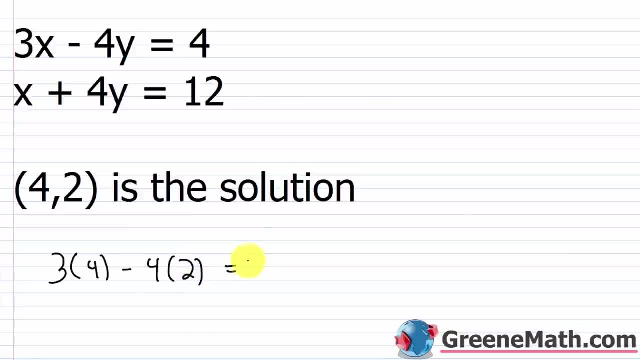 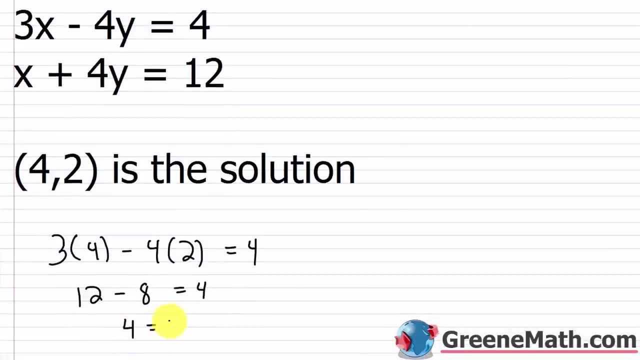 minus 4, plug in a 2 for y, should equal 4. 3 times 4 is 12, minus 4 times 2, that's 8, that should be 4, and it is. You get 4 equals 4. So it works out here. For the second equation, you have x, which I'm plugging in a 4 for x, plus 4 times y, I'm plugging in a 2 for y, is equal to 12. So I get 4 plus 4 times 2 is 8 equals 12, and of course 4 plus 8 is 12, so you get 12 equals 12. 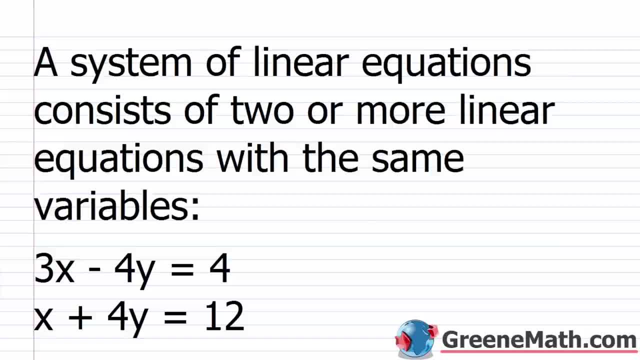 where we start talking about systems of linear equations. So a system of linear equations consists of two or more linear equations with the same variables, And mostly in Algebra 1, we're going to have linear systems that just contain two equations, Two equations with two unknowns. 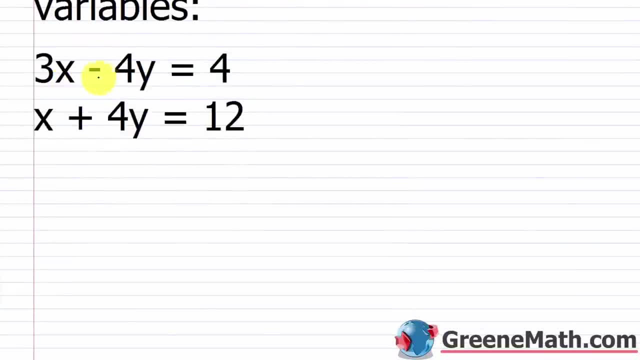 So the first example of this that you're going to see, we have 3x minus 4y equals 4. So it's kind of our first equation. And then we have x plus 4y equals 12. So this right here is known as a system of linear equations. 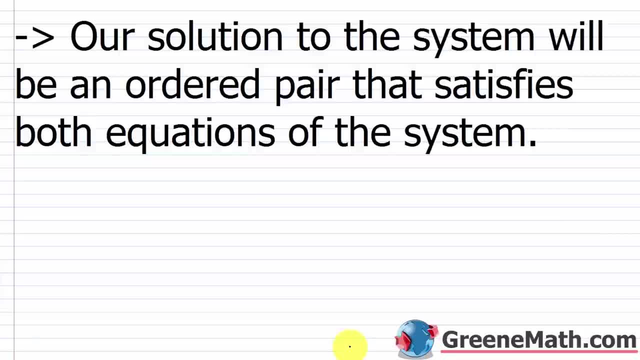 So now our solution is going to be slightly different, because our solution to the system, to the system, will be an ordered pair, and ordered pair that satisfies both equations of this system. So if it's a solution to one but not a solution to the other, it's not a solution to the system. So we're looking for 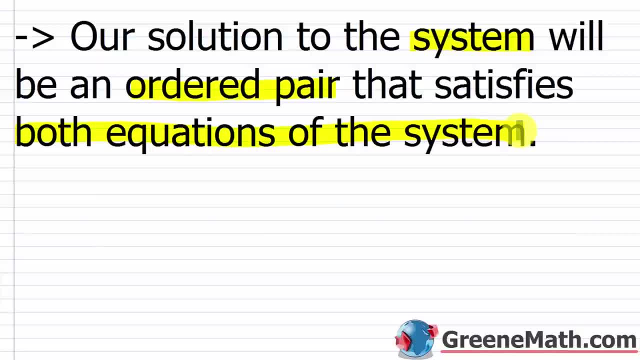 an ordered pair, now that's going to satisfy both equations of that system. Or if you have more than two, let's say all three of the equations of the system, if you had three equations simultaneously. Okay, so that's very, very important, Alright. so here is an example. 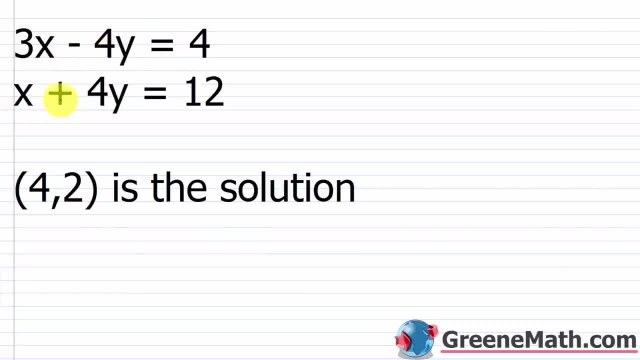 Again we have: 3x minus 4y equals 4, and x plus 4y equals 12.. So I'm giving you the solution. the ordered pair 4 comma 2 is the solution. So the way we check this is the same. We plug a 4 in. 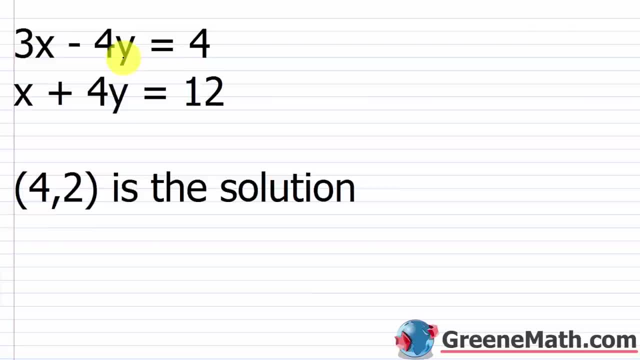 for every x, we plug a 2 in for every y and we make sure the left and the right side are equal in both equations. So for the first one we have 3, plug in a 4 for x minus 4,. plug in a 2 for y. 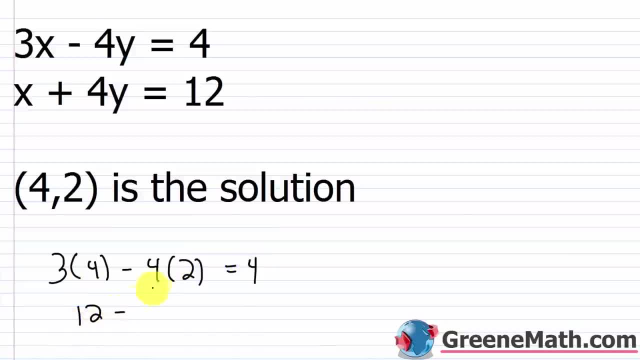 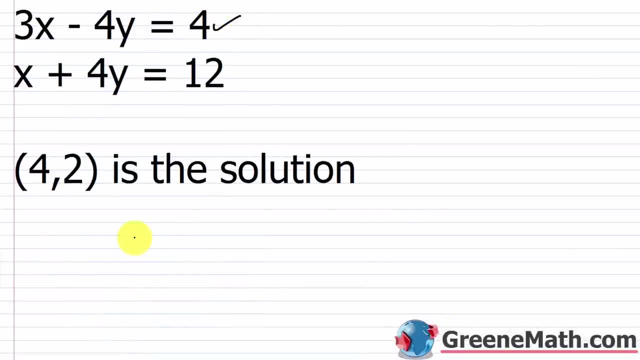 should equal 4.. 3 times 4 is 4.. 12 minus 4 times 2, that's 8, that should be 4, and it is. You get 4 equals 4.. So it works out here. For the second equation, you have x, which I'm plugging in, a 4 for x plus 4 times y. 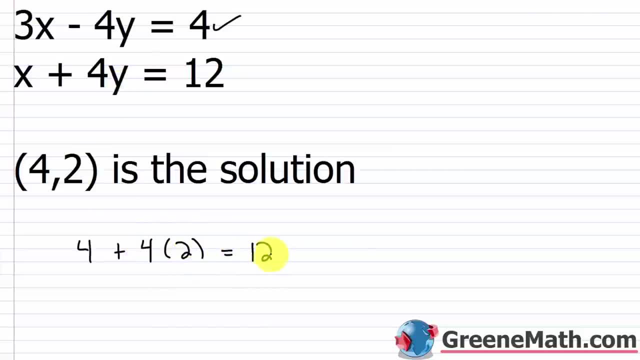 plugging in a 2 for y is equal to 12.. So I get 4 plus 4 times 2 is 8, equals 12, and, of course, 4 plus 8 is 12.. So you get 12 equals 12.. And so, yes, this works out as well. So this ordered pair 4. 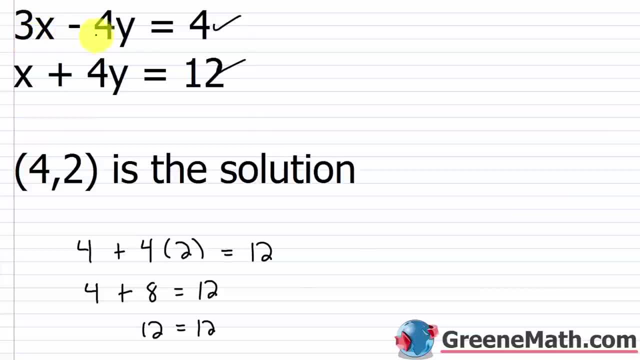 for our system, which again contains the equation 3x minus 4y equals 4, and also x plus 4y equals 12.. Now let's say you had a proposed solution that worked in one but didn't work in the other. 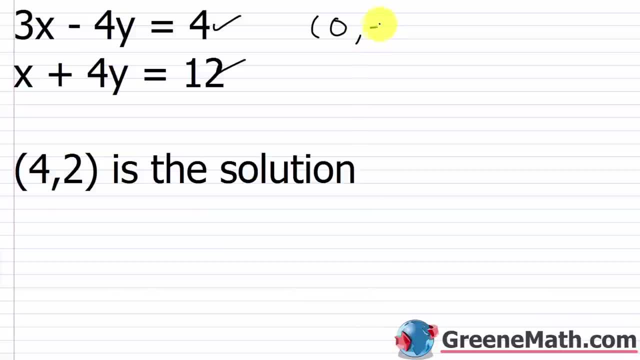 Say you had the ordered pair, 0 comma negative 1.. Is this a solution for the system? Well, it would work. in the first equation, 3 times 0 minus 4 times negative 1 is equal to 4.. That goes away. 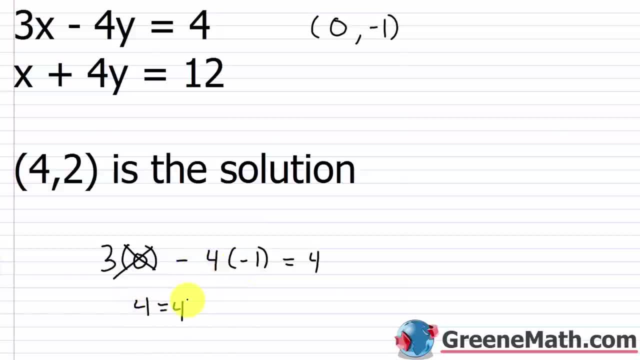 Negative 4 times negative, 1 is 4.. You get 4 equals 4. So that works out. But when you plug it into the second equation it doesn't work. So you'd have a 0 for x plus 4 times negative 1. 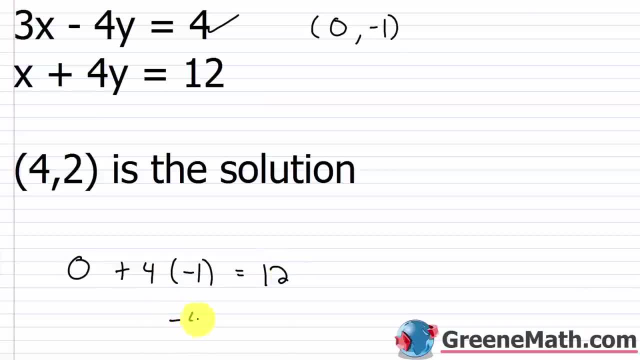 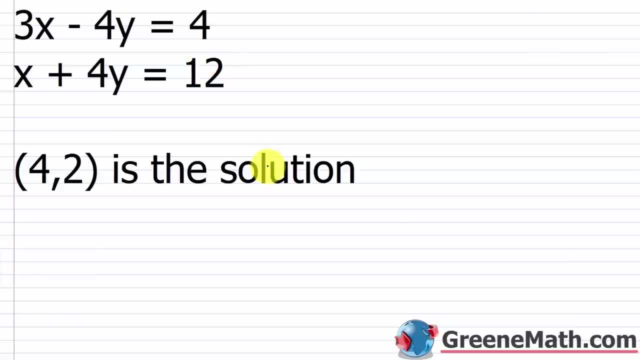 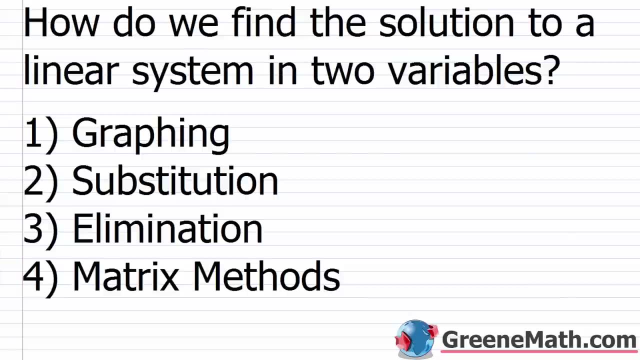 number. It has a number. It has a. this is the heart point. This нашем was smelling like a very small figure, All right, so we can't focus in this one. So our assumption is that whoever did S solved S comprehensively. 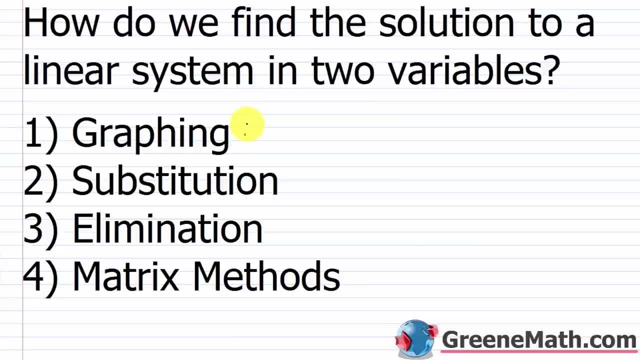 was going to get the one that I'm using in the next one. All right, so when you do S now, or well, once you think about LI maker, whatever that 왜� calls S- You lose This whole piece of one whatsoever to graph, And so you should always use another method. But again, it's something we teach. 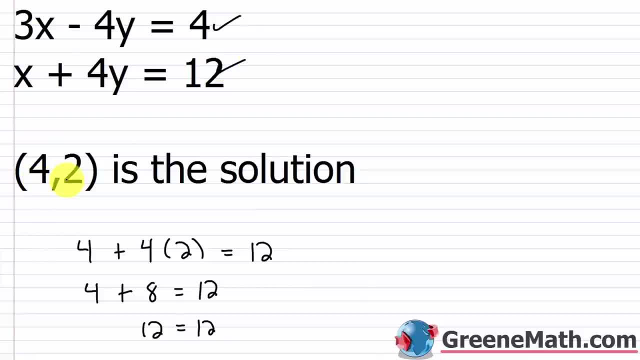 And so yes, this works out as well. So this ordered pair 4 comma 2 is the solution for our system, which again contains the equation 3x minus 4y equals 4, and also x plus 4y equals 12. 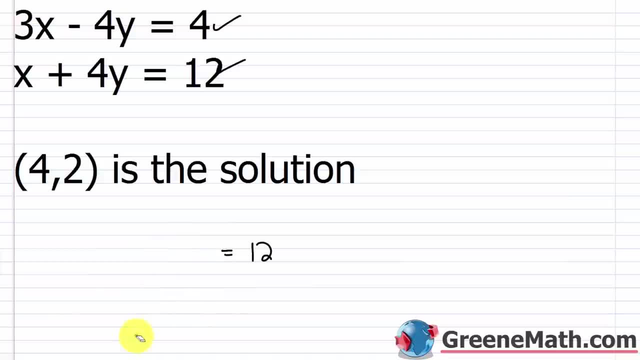 Now, let's say you had a proposed solution that worked in one, but didn't work in the other. Say you had the ordered pair 0 comma negative 1. Is this a solution for the system? 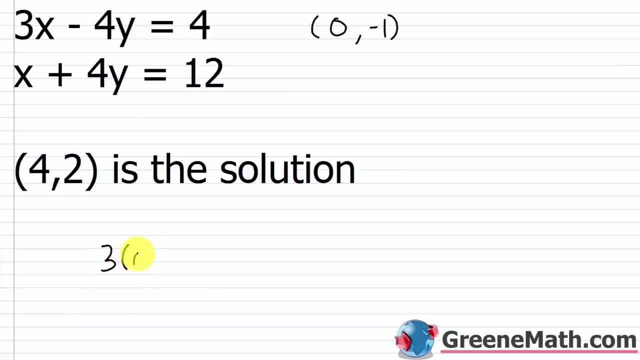 Well, it would work in the first equation, 3 times 0, minus 4 times negative 1 is equal to 4. That goes away. Negative 4 times negative 1 is 4. You get 4 equals 4. So that works out. But when you plug it into the second equation, it doesn't work. So you'd have a 0 for x, plus 4 times negative 1 equals 12. 4 times negative 1 is negative 4. Negative 4 does not equal 12. That's false. So it doesn't work in this one. So this is not a solution to the system. So that's a solution to the system. So that's a solution to the system. 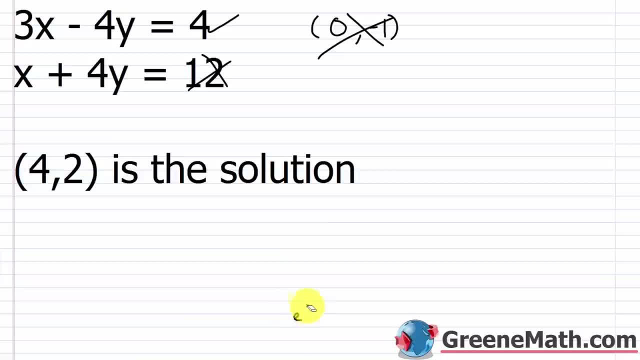 So that's what we mean. We need an ordered pair that works in each equation. It's got to simultaneously solve both of them to be a solution for the system. All right, so how do we find the 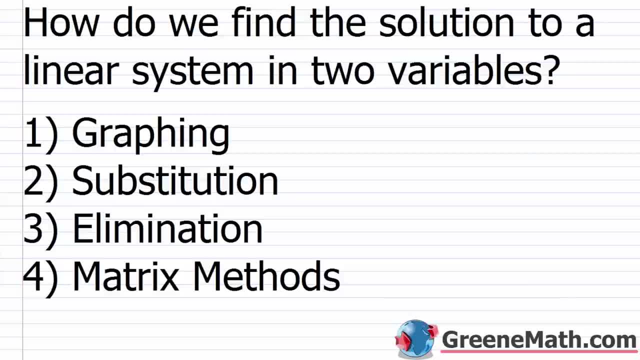 solution to a linear system in two variables? Well, the first thing we're going to do is we're going to learn about graphing. And we're going to talk about that today. Now, graphing is very slow, and it's very inefficient, and it's not something you're going to use. The reason it's even taught is just so you get the concept down. 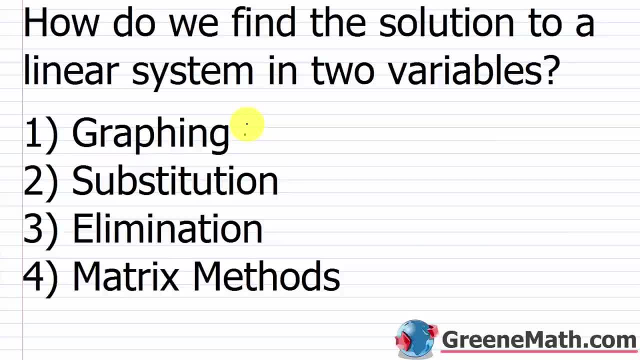 If you have very large or very small values or non-integer values, it makes no sense whatsoever to graph. And so you should always use another method. But again, it's something we teach so that you understand the concept. Now, the next method, which we're going to learn right away, is substitution. Then after that, we're going to learn elimination. And then in algebra 2, we're going to learn some matrix methods. So we're going to cover these three in algebra 1, and then we're going to save this one for algebra 2. 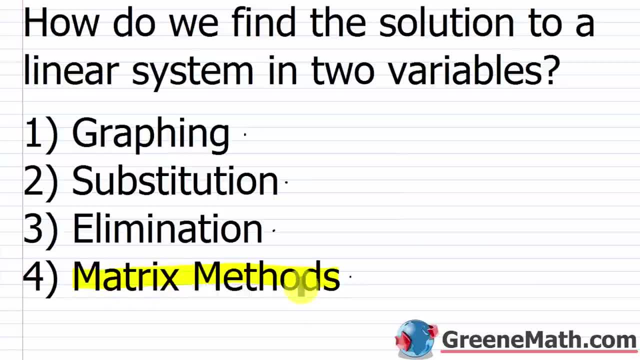 The matrix methods we're going to cover in college algebra. We'll just kind of touch on them in algebra 2, and then we'll really get good in college algebra because the matrix methods are 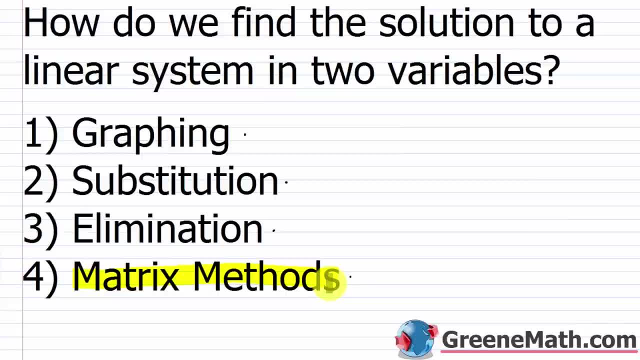 what you're going to use kind of moving forward when you get into higher math to deal with these 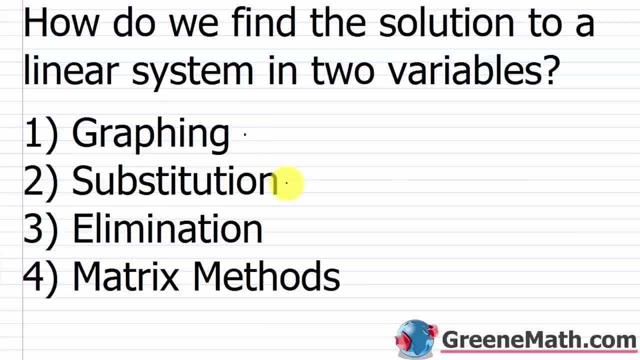 so that you understand the concept. Now, the next method which we're going to learn right away is substitution. Then after that we're going to learn elimination, And then in algebra two we're going to learn some matrix methods. So we're going to cover these three in algebra one. 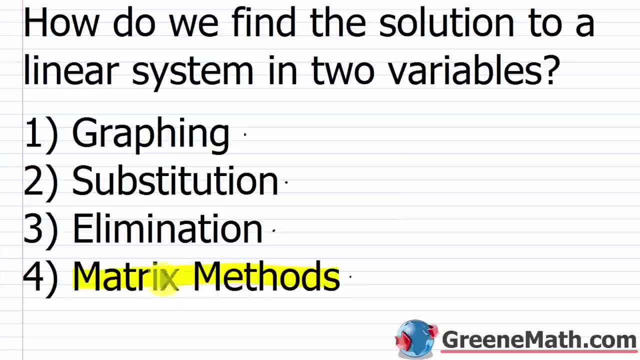 and then we're going to save this one for algebra two And a lot of the matrix methods we're going to cover in college algebra. we'll just kind of touch on them in algebra two And then we'll really get good in college algebra because the matrix methods are what you're going to use kind. 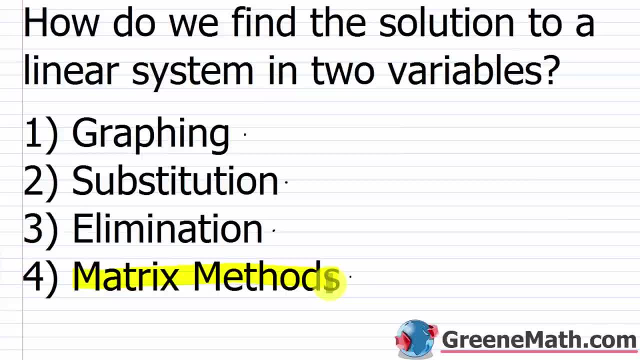 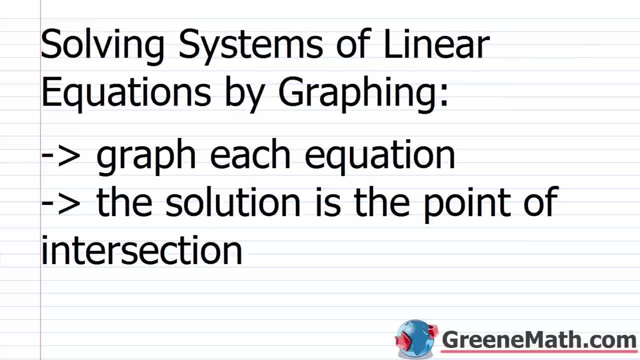 of moving forward when you get into higher math, to deal with these really, really big systems. Alright, so I have here. let's start by learning the least efficient method: graphing. Alright, so it's actually very, very easy to solve a system of linear equations by. 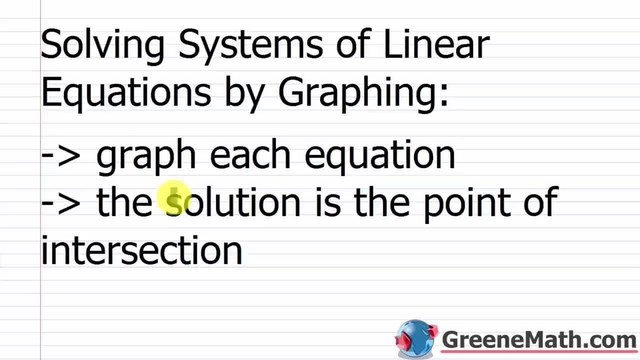 graphing. You just simply graph each equation And then the solution is the point of intersection. Okay, again, the solution is the point of intersection. And why do you think that is? Well, if we kind of just think about this logically, if I graph a linear equation, I have a line. let's say this is the. 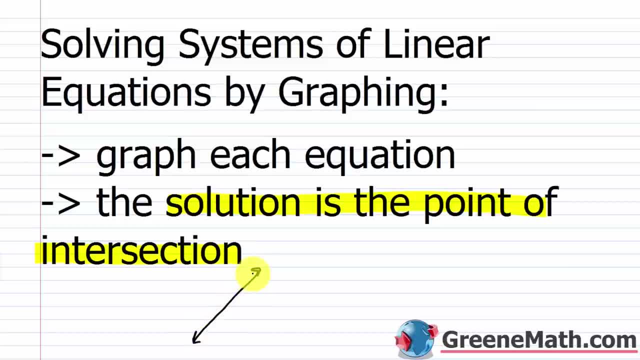 line here. Every point on that line is a solution to the equation. If I graph another linear equation, let's say this is another line, every point on this is also a solution for the other equation. So that point of intersection- right, there is a solution to the equation. So if I 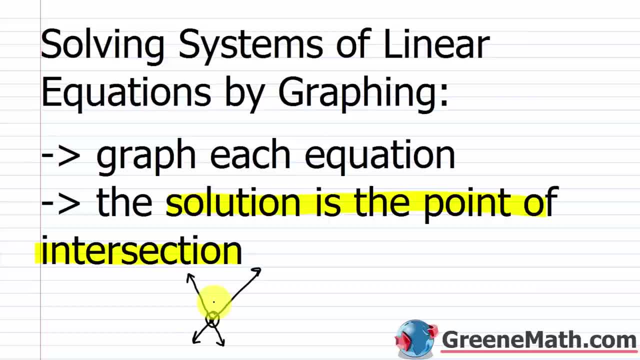 graph, another linear equation. let's say: this is another line. every point on this is also a solution to both Right. it solves the first one and it solves the second one because that point is on each line And so therefore it is a solution to both equations. So let's go ahead and take a look. 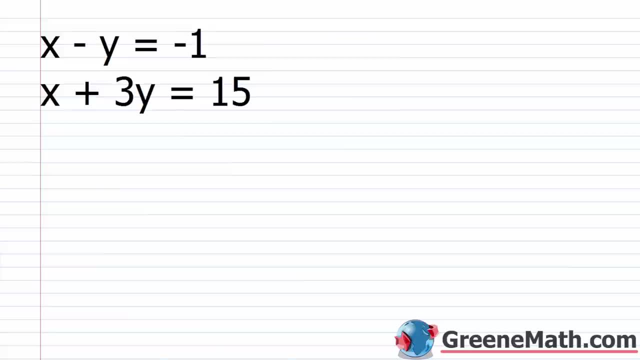 at the first problem. So we have x minus y equals negative one, and we have x plus three, y equals 15. So very easy to graph. at this point we know all the tricks. we're going to solve each for y, put it in slope intercept form and we're going to graph them very quickly. So to solve this for y, 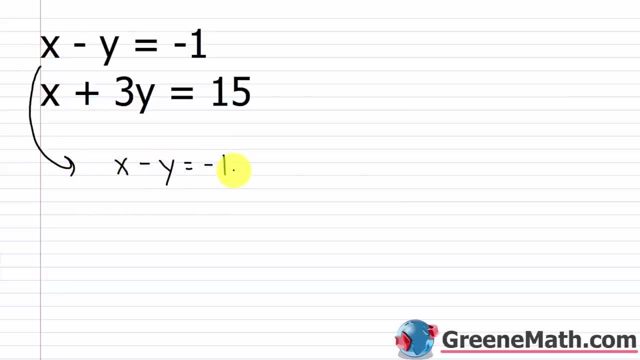 I'd have: x minus y equals negative one. I'm going to subtract x away from each side. then I have negative y is equal to negative x minus one. multiply both sides of the equation by negative one. I'm going to get y is equal to x plus one. Okay, for the next one again. 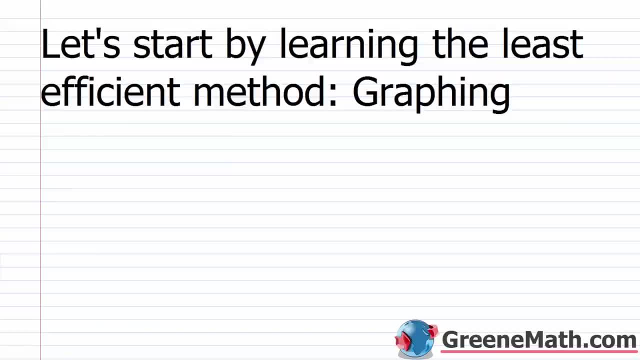 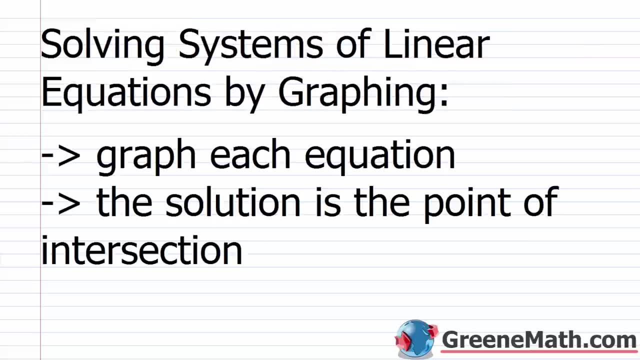 really, really big systems. All right, so I have here, let's start by learning the least efficient method, graphing. All right, so it's actually very, very easy to solve a system of linear equations by graphing. You just simply graph each equation, and then the solution is the point of intersection. 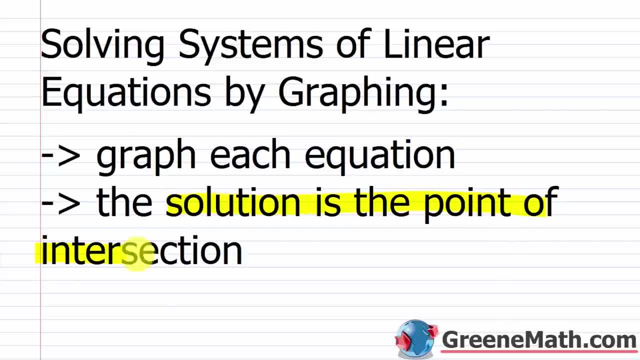 Okay, again, the solution is the point of intersection. And why do you think that is? Well, if we kind of just think about this, logically, if I graph a linear equation, I have a line. Let's say this is the line here. Every point on that line is a solution to the 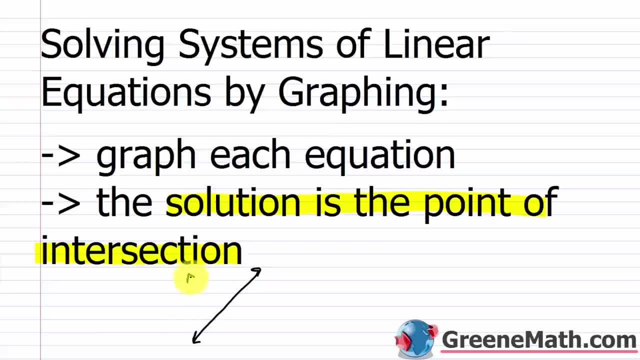 equation. If I graph another linear equation, let's say this is another line, every point on this is also a solution for the other equation. So that point of intersection right there, is a solution to both, right? It solves the first one, and it solves the second one, because 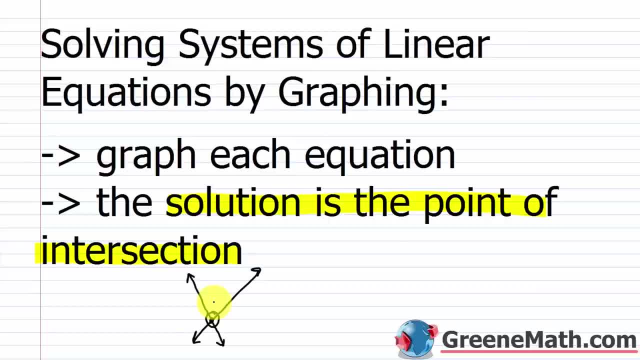 that point is on each line. And so therefore, it is a solution to both equations. So let's go ahead 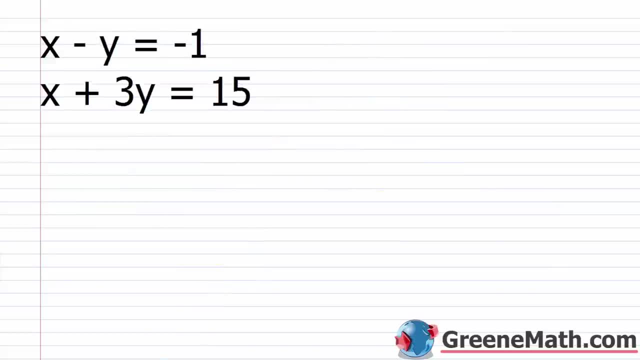 and take a look at the first problem. So we have x minus y equals negative one, and we have x plus 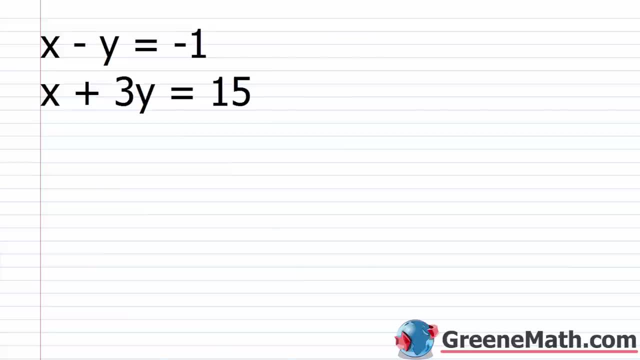 three y equals 15. So very easy to graph at this point. We know all the tricks. We're going to solve each for y, put it in slope-intercept form, and we're going to graph them very quickly. 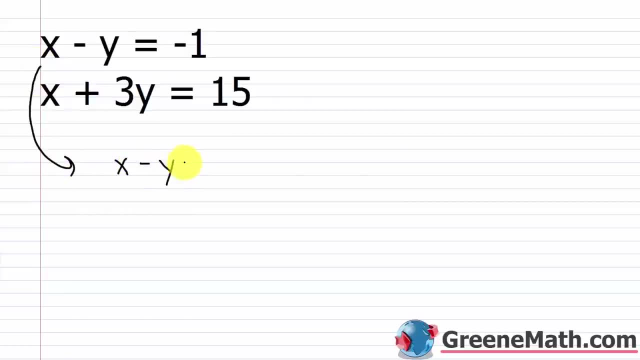 So to solve this for y, I'd have x minus y equals negative one. I'm going to subtract x away from each side. Then I have negative y is equal to negative x minus one. Multiply both sides of the equation by negative one. I'm going to get y is equal to x plus one. 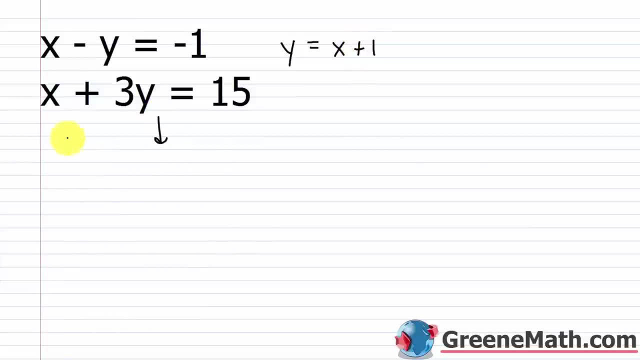 Okay, for the next one, again, I want to solve this for y. So I'm going to subtract, I'm going to subtract x, 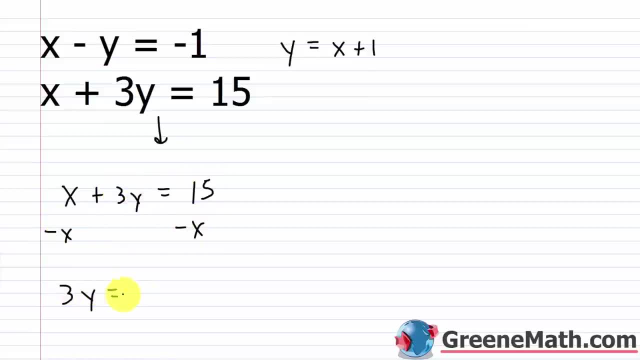 I'm going to subtract y is equal to negative x plus 15, and then just divide each side by three. And that's going to give me what? Let's erase this, and I'd have negative one-third x, 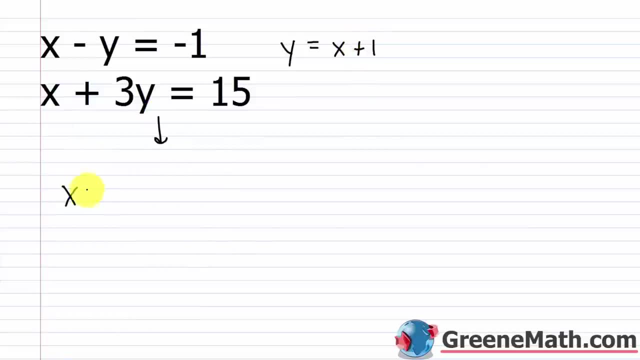 I want to solve this for y, So I'm going to subtract. I'm going to subtract x away from each side, So I'd have three: y is equal to negative x plus 15.. And then just divide each side by three And that's going to give me what. let's erase this And I'd have negative one third x. 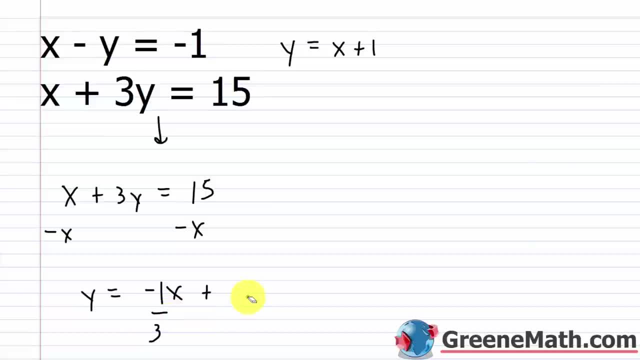 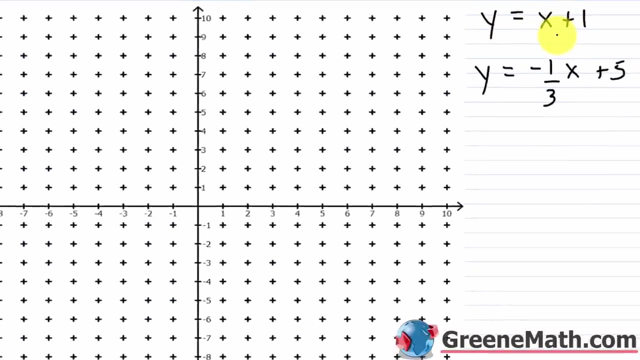 kind of write it like this: Plus 15 over three is five. So y is equal to negative one third x plus five. So let's take these two down to the coordinate plane, Alright, so we have y equals plus one. So we know the y intercept will occur at zero comma one. So that's right there. 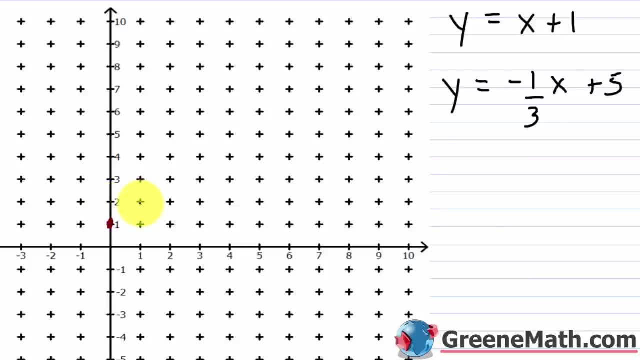 And the slope is going to be one. So I go up one and over one, up one and over, up one and over one, or I can go down one into the left, one down one into the left one down one into the left one. 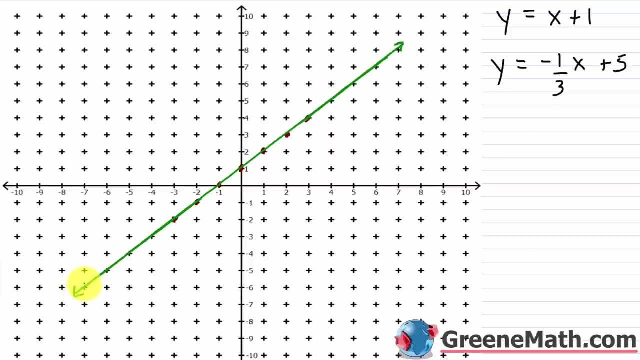 Okay, This is: y equals x plus 1.. All right now for y equals negative 1 third x plus 5, the y-intercept is going to occur at 0 comma 5.. So that's going to be right here. 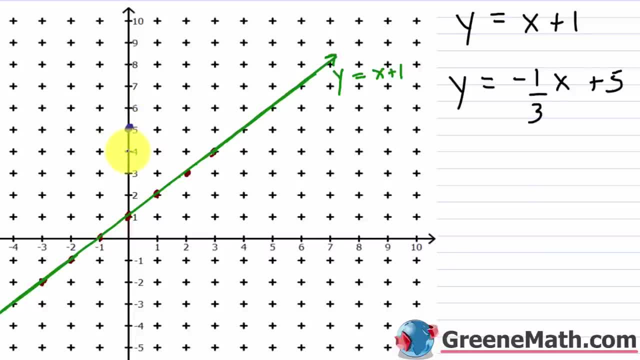 And the slope is negative 1 third. So that means I would fall 1 and go to the right- 1,, 2,, 3.. And I've found my point of intersection already: Fall 1,, go to the right- 1,, 2,, 3.. 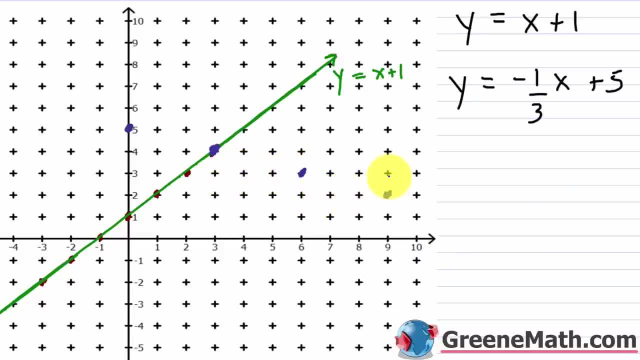 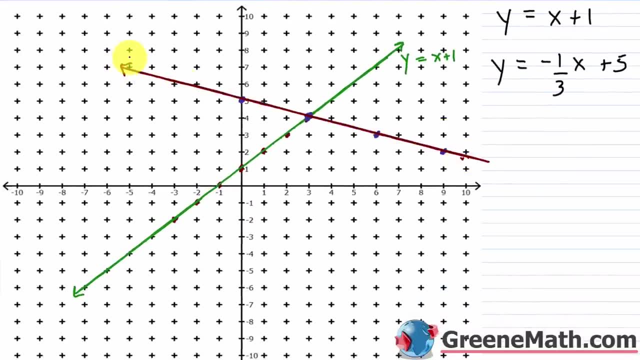 Fall 1, go to the right: 1,, 2,, 3. And let's go ahead and graph this guy. Okay, so this point, right here, is your point of intersection, So that ordered pair lies on both lines. So therefore it's a solution to the system. 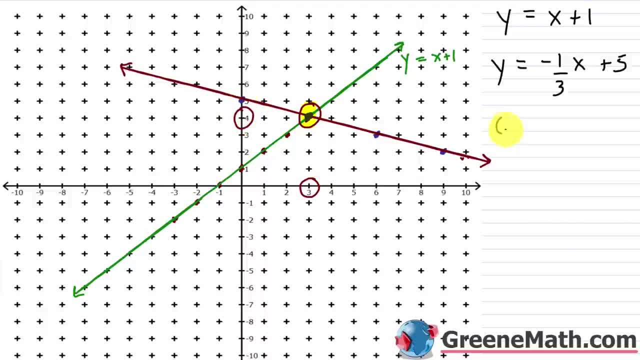 And so that's going to be the point 3 comma 4.. 3 comma 4.. And that's another problem with graphing. If you don't graph that well, if you don't have a ruler or you can't get an accurate graph going, 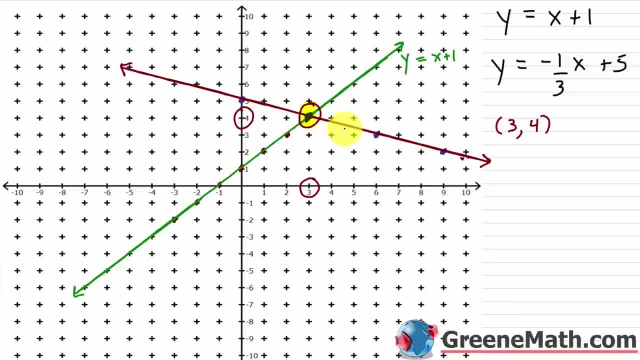 it's kind of hard to graph, It's kind of hard to tell where it intersects. I mean, here it's pretty obvious. I chose a problem. that would be very easy. But if you had a real-world problem or you had a problem, that's kind of going to come later on in your textbook. 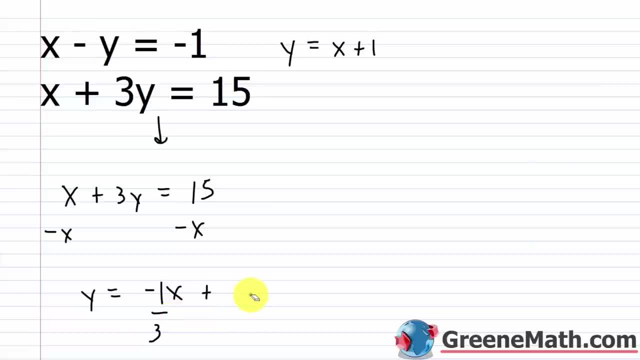 kind of write it like this, plus 15 over three is five. So y is equal to negative one-third x plus five. So let's take these two down to the coordinate plane. All right, so we have 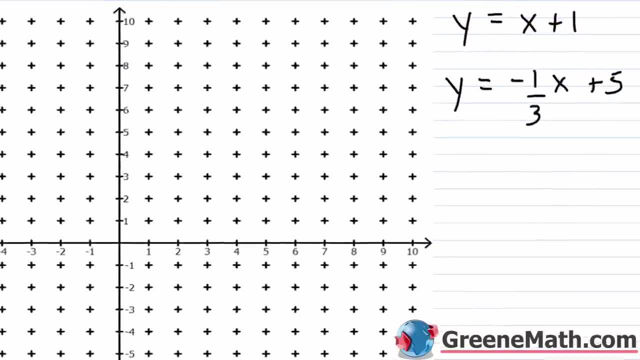 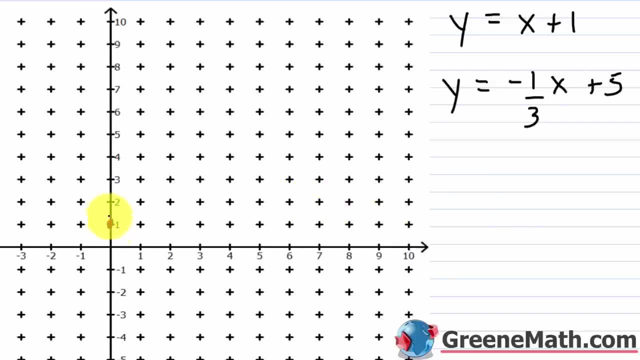 y equals x plus one. So we know the y-intercept will occur at zero comma one. So that's right there. And the slope is going to be one. So I go up one and over one, up one and over one, up one and over one. Or I can go down one and to the left one, down one and to the left one, down one and to the left one. 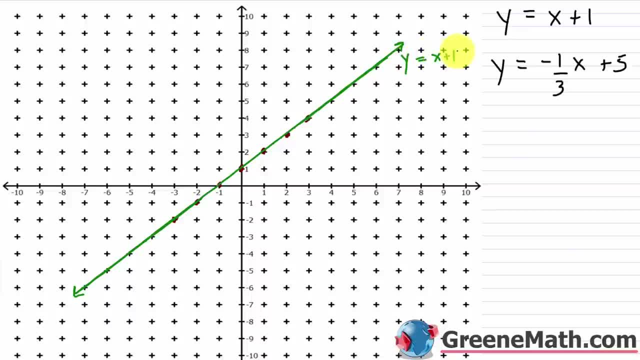 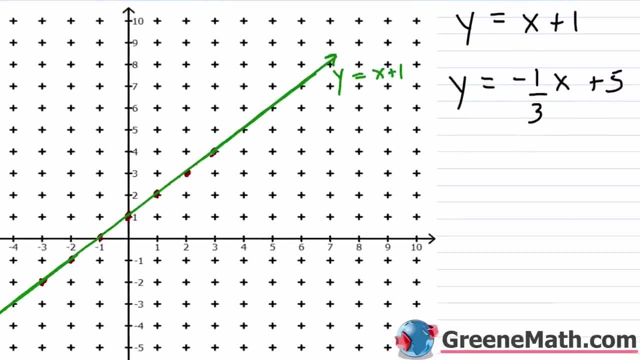 Okay, so this is y equals x plus one. All right, now for y equals negative one-third x plus five, the y-intercept is going to occur at zero comma five. So that's going to be right here. And the slope is negative one-third. So that means I would fall one and go to the right one, two, three. And I've found my point of intersection already. Fall one, go to the right one, two, three. Fall one, go to the right one, two, three. And let's go ahead and graph this. This guy. 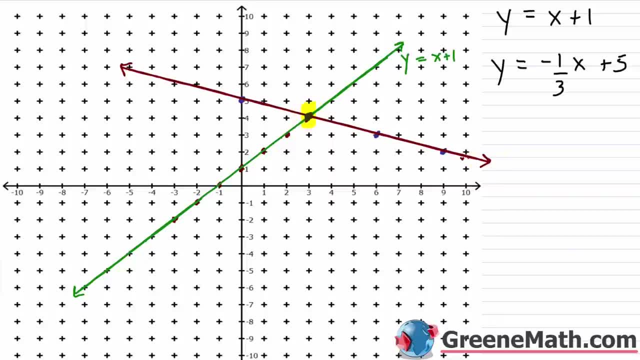 Okay, so this point right here is your point of intersection. So that ordered pair lies on both lines. So therefore, it's a solution to the system. And so that's going to be the point three comma four, three comma four. And that's another problem with graphing. If you don't graph that well, if you don't have a ruler or you can't get an accurate graph, you can't get an accurate graph. So that's going to be the point three comma four. 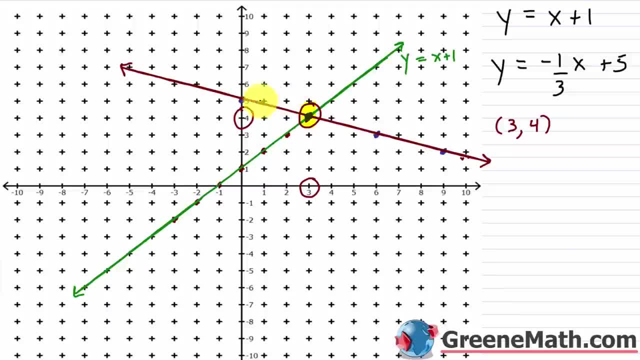 It's kind of hard to tell where it intersects. I mean, here it's pretty obvious. I chose a problem that would be very easy. But if you had a real world problem where you had a problem that's kind 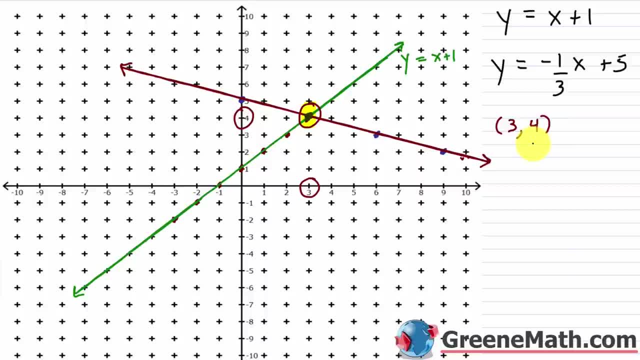 of going to come later on in your textbook, it would be really, really difficult to get an answer. So let's go back up and let's check that proposed solution of three comma four. 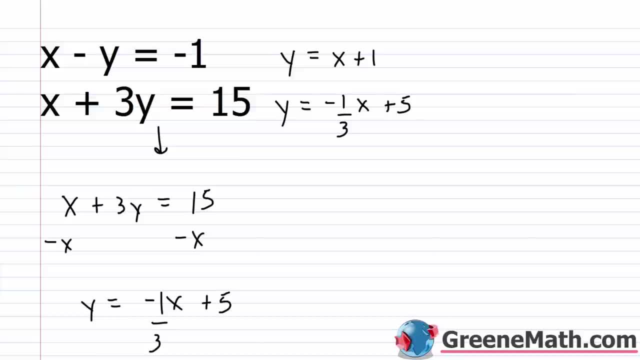 it would be really, really difficult to get an answer. So let's go back up And let's check that proposed solution of 3 comma 4.. So we're saying that's our solution, The ordered pair: 3 comma 4.. 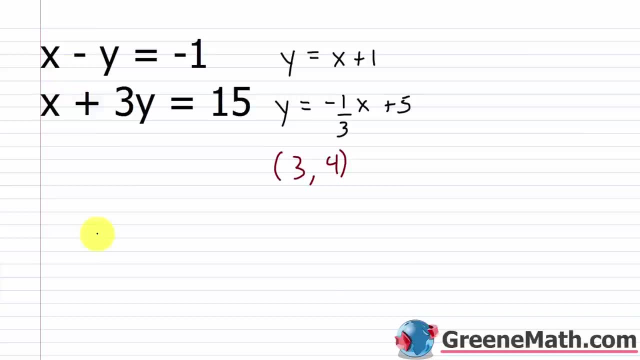 Let's check it in the original equation. So in the first equation I have x minus y equals negative 1.. So that would be 3 minus 4 equals negative 1.. Of course that's true. You get negative 1 equals negative 1.. 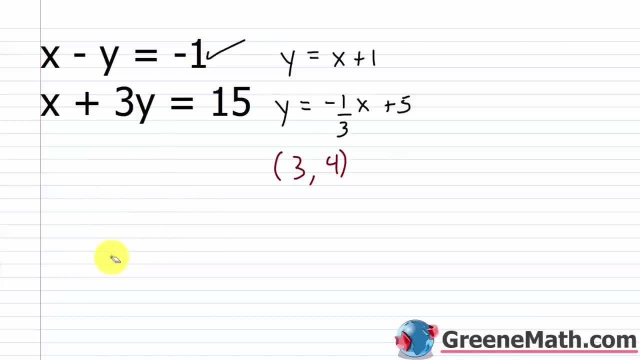 So it works there. In the second equation I've got: x plus 3y equals 15. So I'm plugging in a 3 for x plus 3 times for y. I'm plugging in a 4. And this equals 15.. 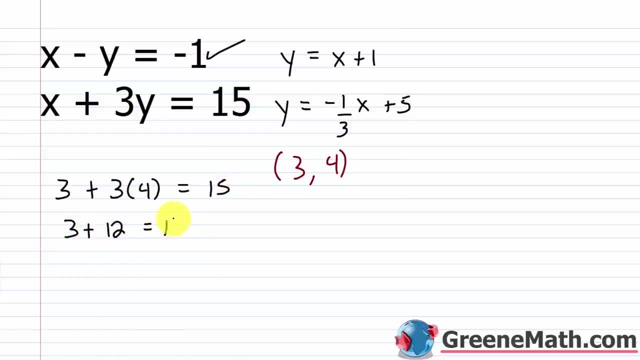 So 3 plus 3 times 4 is 12 equals 15. And you get 15 equals 15.. So it checks out there as well. So 3 comma 4, that ordered pair is a solution for this system. 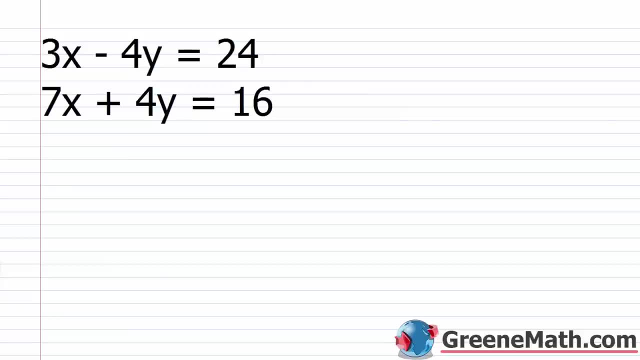 All right, let's take a look at another example. We have 3x minus 4y equals 24.. We have 7x plus 4y equals 16.. So again, I'm going to solve each one for y. 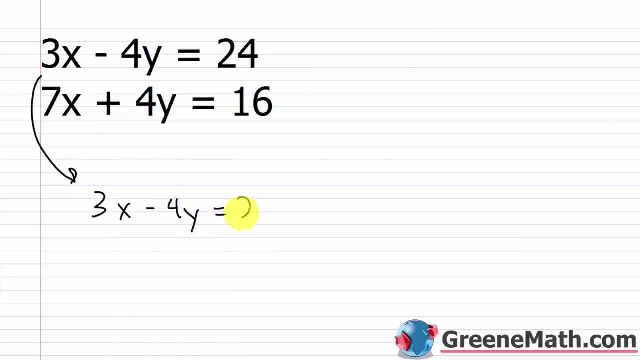 So 3x minus 4y equals 24.. I'm going to subtract 3x away from each side I'll have negative. 4y is equal to negative 3x plus 24.. I'm going to divide each side by negative 4.. 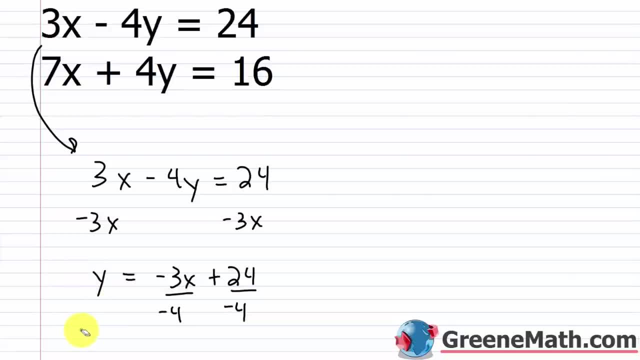 And so this is going to cancel. I'll just have y. Negative 3 over negative 4 is just 3 fourths. I'll get rid of the negatives. I'll just write this as 3 fourths times x, And then plus 24 over negative 4, that's going to be minus 6.. 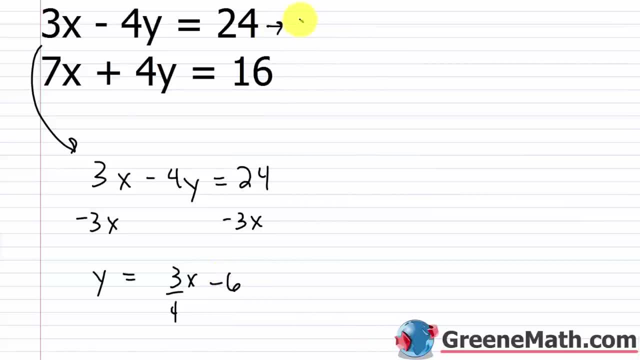 So this guy right here, if I write it in slope-intercept form, is: y equals 3 fourths x minus 6.. For the next one, we're also going to solve for y, So I'm going to subtract 7x away from each side. 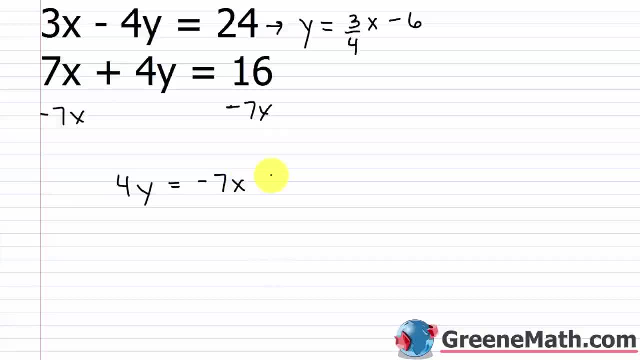 I'll have: 4y is equal to negative 7x plus 16.. Divide each side by 4.. And get: y is equal to negative 7 fourths x plus 4.. So this is: y is equal to negative 7 fourths x plus 4.. 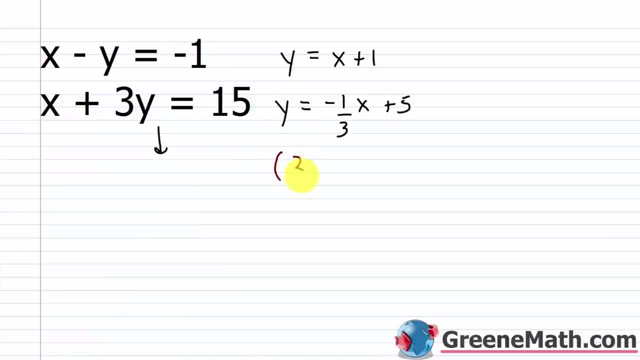 So we're saying that's our solution. The ordered pair three comma four. Let's check it in the ness equation. So we're saying that's our solution. That's our solution. And the answer is, three comma four equals negative one. And of course, we don't have a solution that's going to be a correct answer. So what we're saying is that it's positive. So this is what we're saying is, three minus four equals negative one. So that would be three minus four equals negative one. 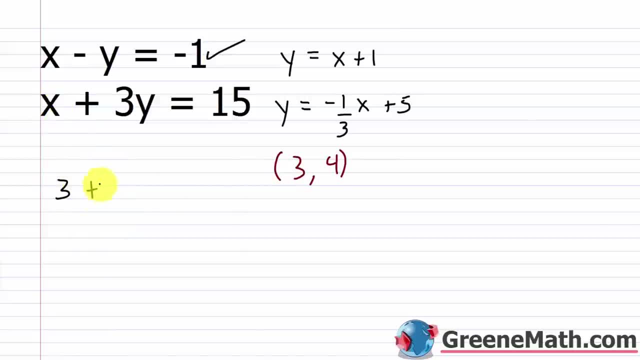 Of course, that's true. You get negative one equals negative one. So it works there. In the second equation, I've got x plus three y equals 15. So I'm plugging in a three for x, plus three times for y, I'm plugging in a four. And this equals 15. So three plus three times four is 12 equals 15. And you get 15 equals 15. So checks out there as well. So three comma four, 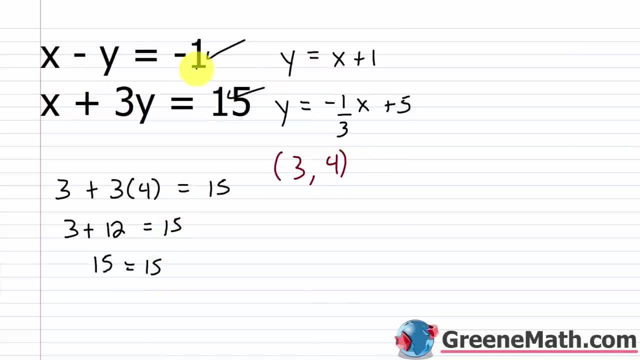 4, that ordered pair, is a solution for this system. Well, let's take a look at another example. 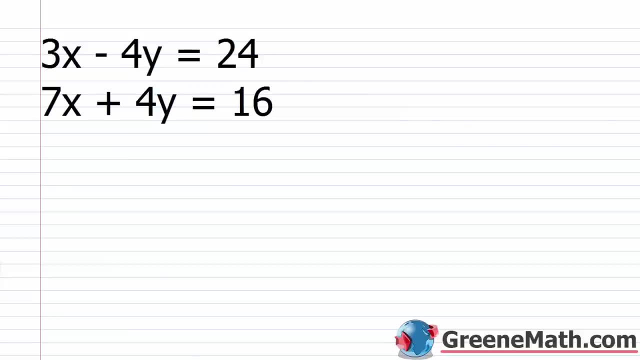 We have 3x minus 4y equals 24. We have 7x plus 4y equals 16. So again, I'm going to solve each one for y. So 3x minus 4y equals 24. I'm going to subtract 3x away from each side. I'll have negative 4y is equal to negative 3x plus 24. I'm going to divide each side by negative 4. 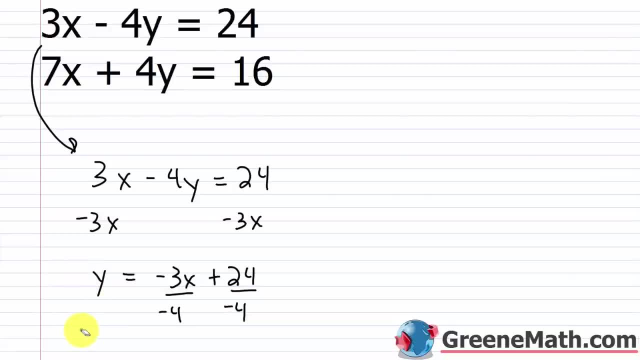 And so this is going to cancel. I'll just have y. Negative 3 over negative 4 is just 3 fourths. 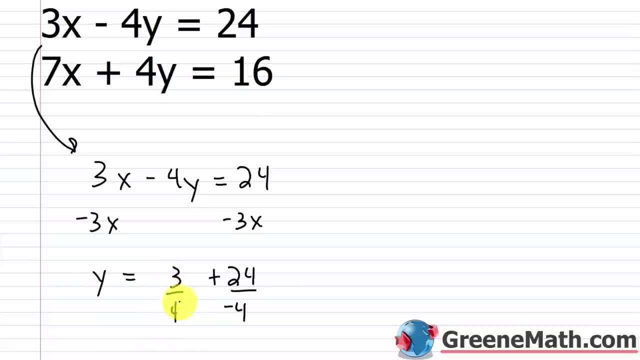 I'll get rid of the negatives. I'll just write this as 3 fourths times x. And then plus 24 over negative 4, that's going to be minus 6. So this guy right here, if I write it in slope-intercept form, is y equals 3 fourths x minus 6. For the next one, we're also going to solve for y. 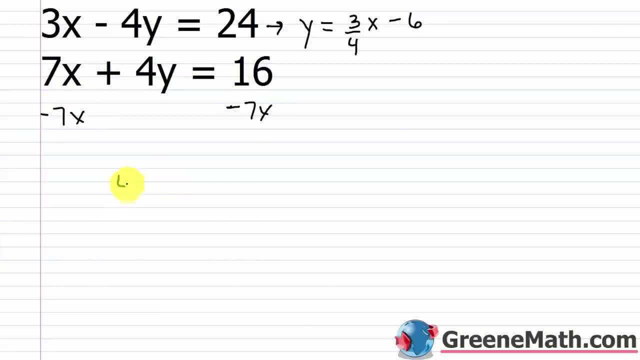 So I'm going to subtract 7x away from each side. I'll have 4y is equal to negative 7x plus 16. Divide each side by 4 and get y is equal to negative 7 fourths x plus 4. So this is y is 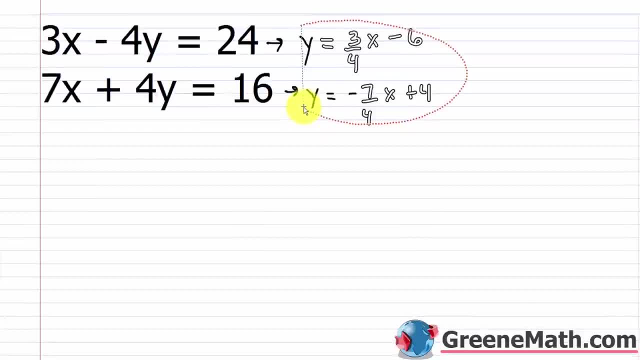 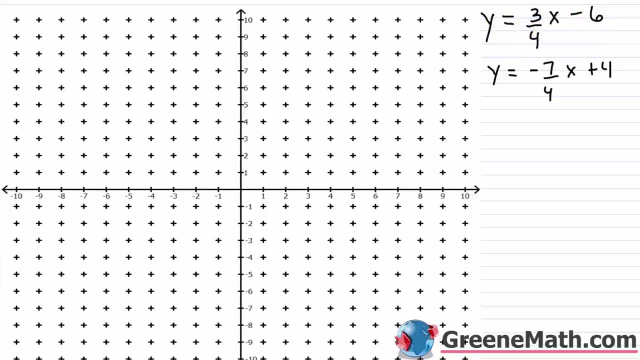 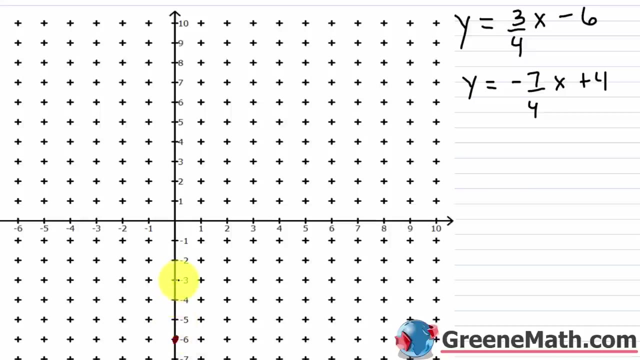 Alright, let's go ahead and take this down to the coordinate plane. Alright, so we have each equation solved for y. Very easy to graph it. The first one, y equals 3 fourths x minus 6. The y intercept will occur at 0 comma negative 6. The slope is 3 fourths. So up 3, 1, 2, 3, to the right 4. 1, 2, 3, 4. Up 3, 1, 2, 3, to the right 1, 2, 3, 4. 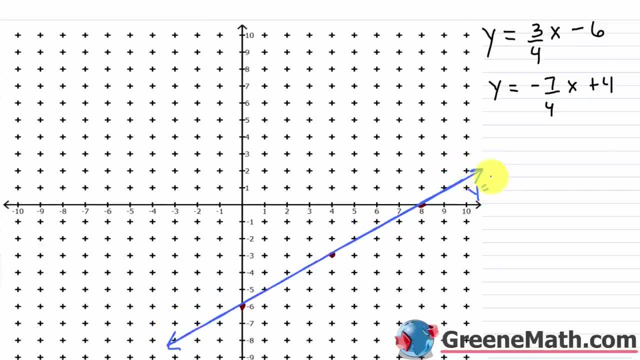 So this one is y equals 3 fourths x minus 6. I'll just always label the first one. Once we put the 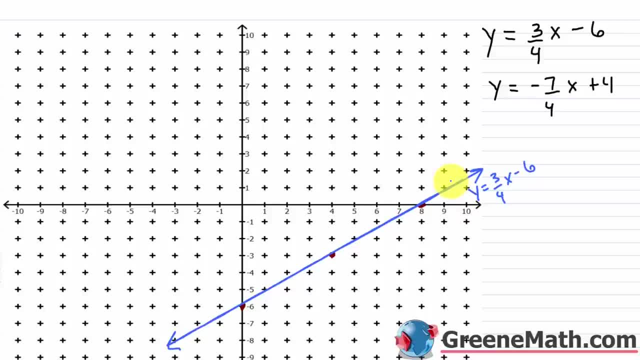 second one in, we don't really need to label it. Just try to not get confused. So we now have y 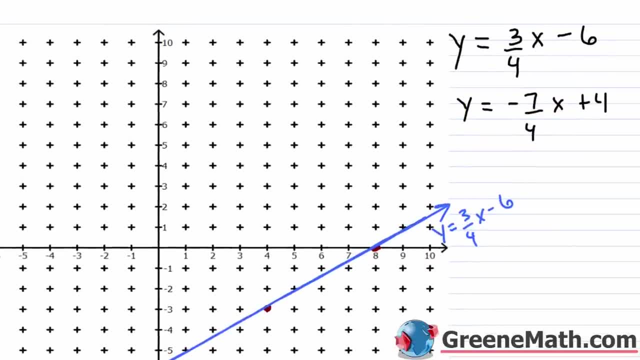 equals negative 7 fourths x plus 4. So that has a y intercept at 0 comma 4 and a slope of negative 7 fourths. So I'm going to go down 7. I'm going to go down 1, 2, 3, 4, 5, 6, 7 to the right 4. 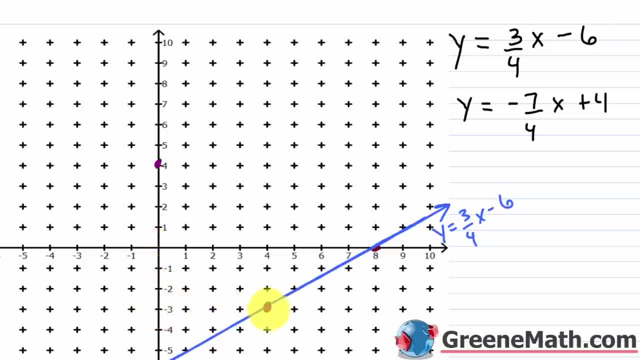 1, 2, 3, 4. And we see we have, again, a point of intersection already. Now if I go down 7 again, I'm going to go to the very bottom part of my graph. So I'm going to go down 1, 2, 3, 4, 5, 6, 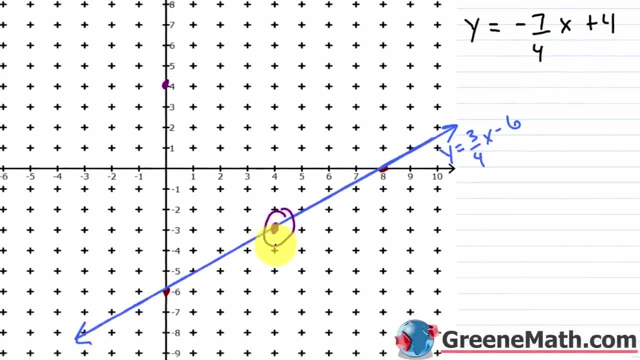 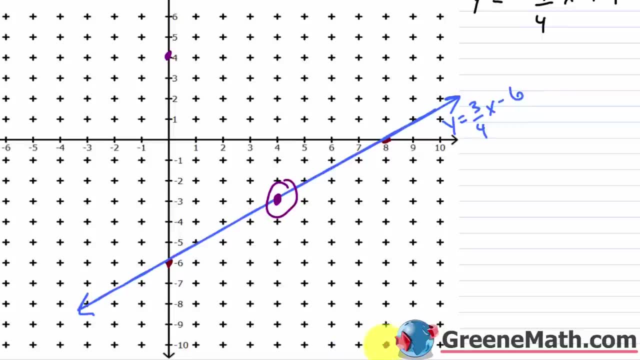 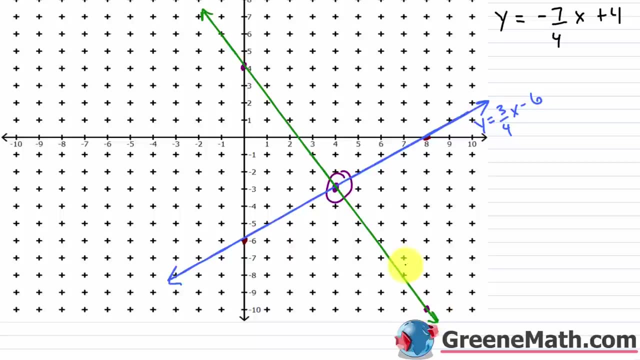 7 to the right 1, 2, 3, 4. So you can label this second one if you want. Just go ahead and put y 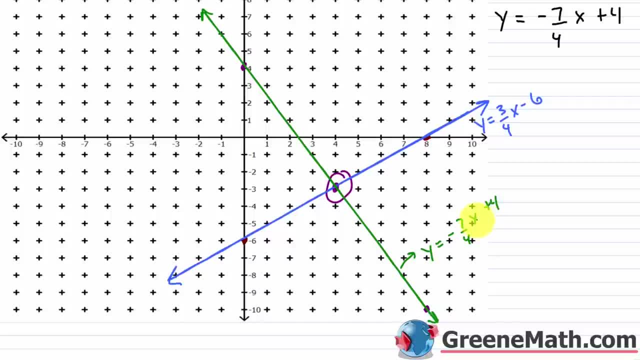 equals negative 7. So you can label this second one if you want. Just go ahead and put y equals negative 7. So you can label this second one if you want. Just go ahead and put y equals negative 7 fourths x plus 4. You don't have to label these. In the previous example, I didn't even 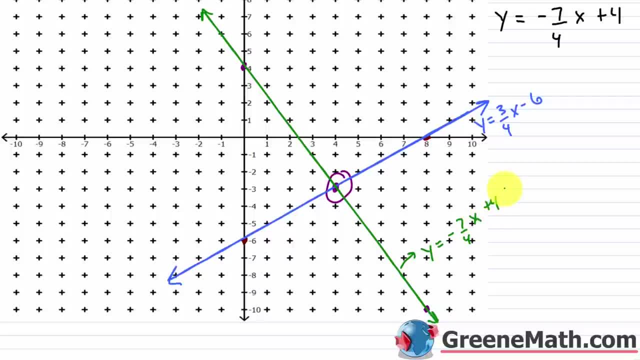 label the second one. Sometimes it's a good idea just when you first start out to not get confused about which equation was which. But the ultimate goal here, we already know how to graph. We've 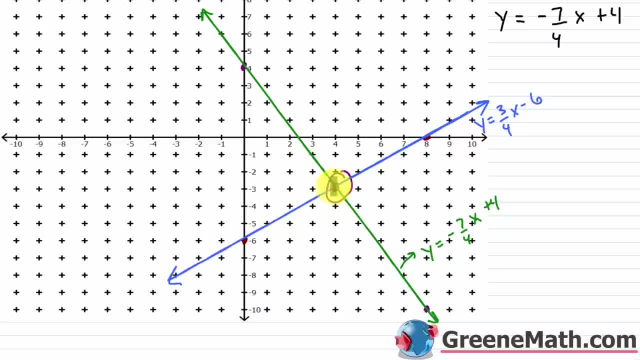 already figured that out in kind of the last section of Algebra 1. Now we're just looking for the point of intersection between the two lines. And in this case, it's very easy to find. 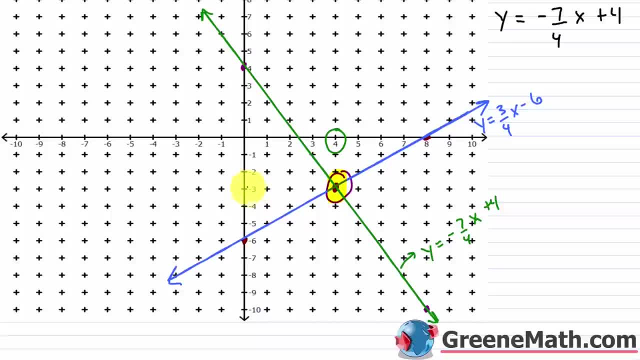 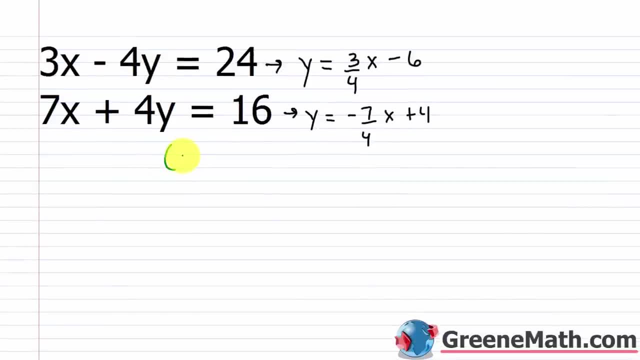 It's at the ordered pair 4 for x and negative 3 for y. So 4 comma negative 3. So let me put that down. The ordered pair is 4 comma negative 3. 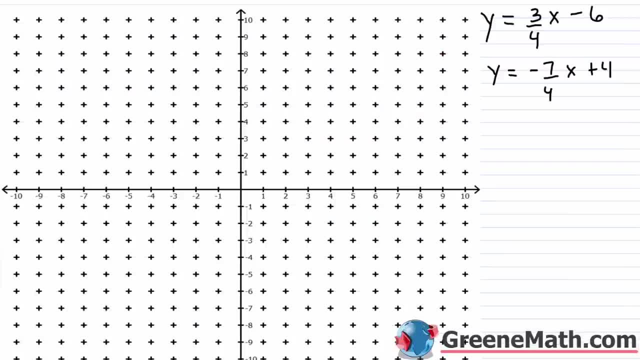 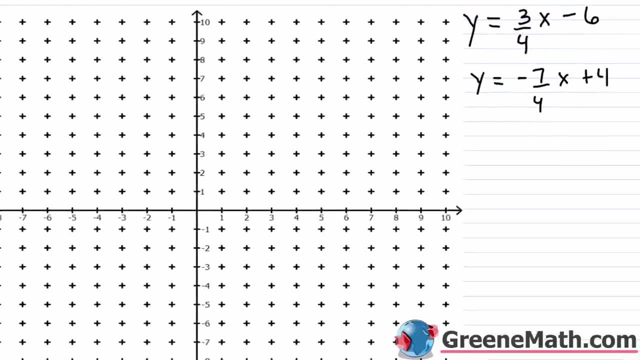 All right, let's go ahead and take this down to the coordinate plane. All right, so we have each equation solved for y. Very easy to graph it. The first one, y, equals 3 fourths x minus 6.. The y-intercept will occur at 0 comma negative 6.. 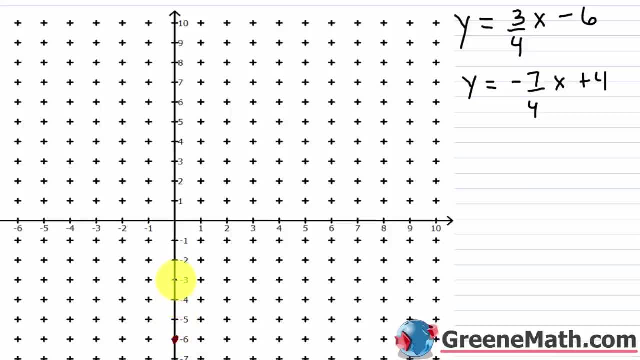 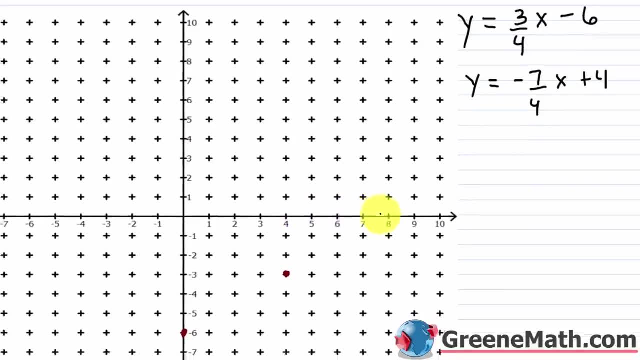 The slope is 3 fourths. So up 3, 1,, 2,, 3, to the right, 4. 1,, 2,, 3, 4.. Up 3, 1,, 2,, 3, to the right. 1,, 2,, 3,, 4.. 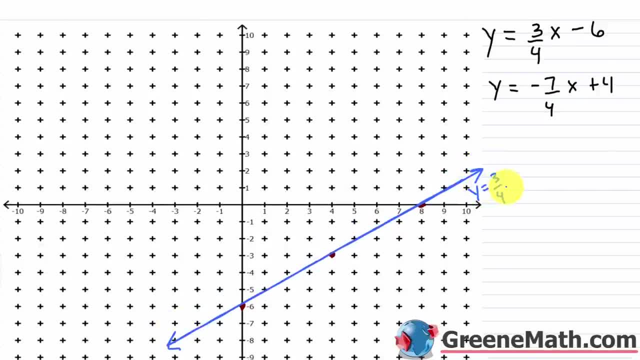 So this one is: y equals 3 fourths x minus 6.. Now I'll just always write this as 3 fourths x minus 6.. I'll just always label the first one. Once we put the second one in, we don't really need to label it. 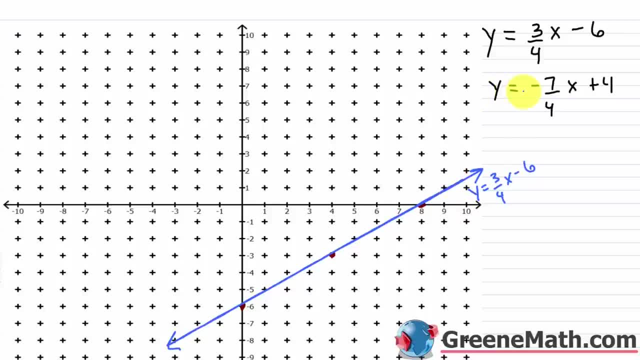 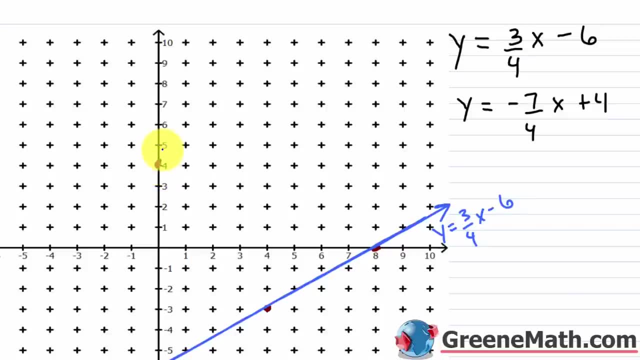 Just try to not get confused. So we now have y equals negative 7 fourths x plus 4. So that has a y-intercept at 0 comma 4 and a slope of negative 7 fourths. So I'm going to go down 7.. 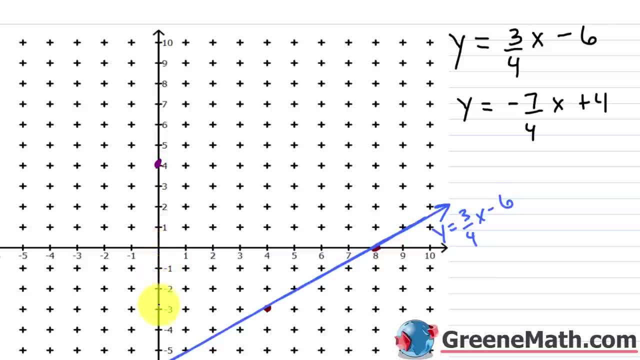 I'm going to go down: 1,, 2,, 3,, 4,, 5,, 6,, 7 to the right, 4.. 1,, 2,, 3,, 4.. And we see we have again a point of intersection already. Now, if I go down 7, I'm going to go down 1,, 2,, 3,, 4,, 5,, 6,, 7 to the right, 4.. 1,, 2,, 3,, 4.. 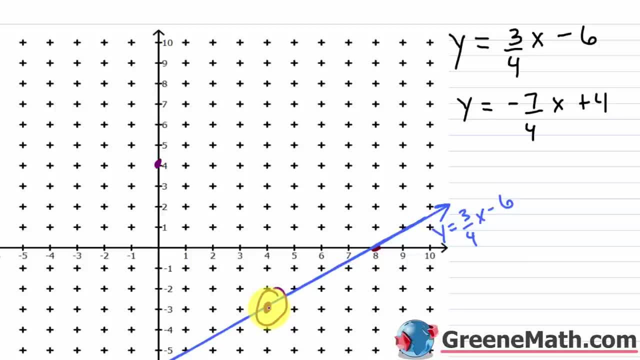 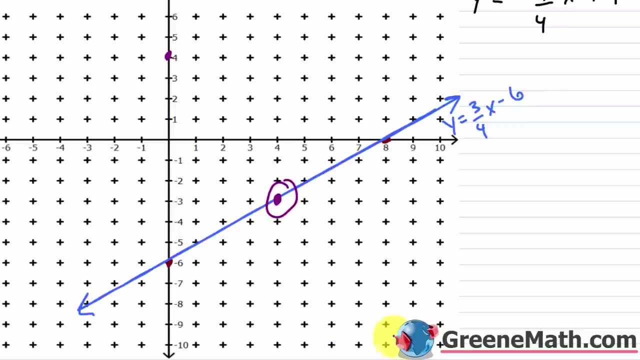 1,, 2,, 3, 4.. 1,, 2,, 3, 4.. Now, if I go down 7 again, I'm going to go to the very bottom part of my graph. So I'm going to go down 1,, 2,, 3,, 4,, 5,, 6,, 7 to the right: 1,, 2,, 3, 4.. 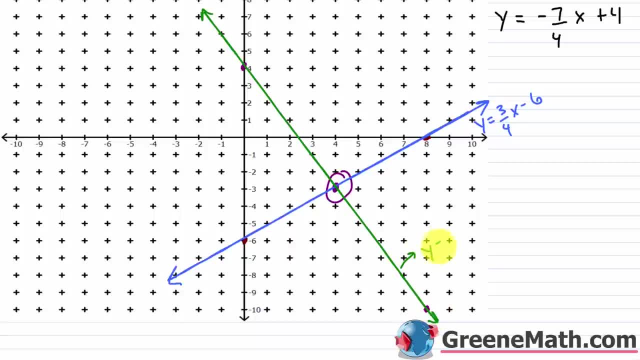 So you can label the second one. if you want, Just go ahead and put: y equals negative 7 fourths x plus 4.. You don't have to label these. In the previous example I didn't even label the second one. Sometimes it's a good idea. 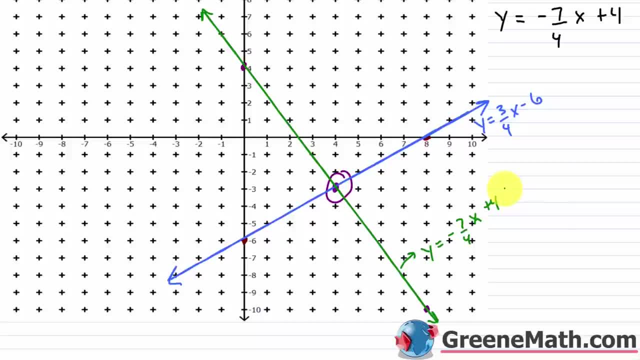 Just when you first start out, to not get confused about which equation was which. But the ultimate goal here we already know how to graph. We've already figured that out in kind of the last section of Algebra 1.. Now we're just looking for the point of intersection between the two lines. 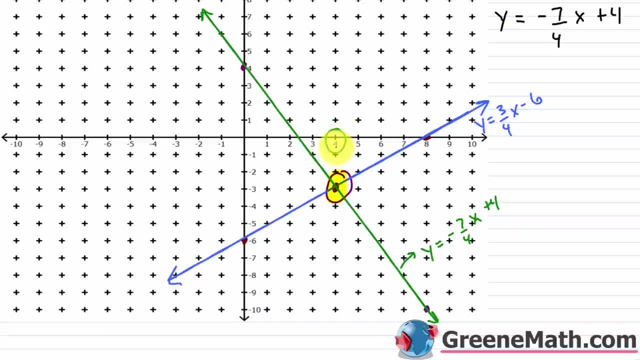 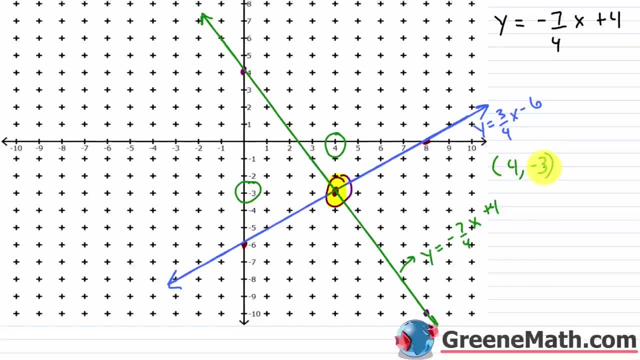 And in this case it's very easy to find- It's at the ordered pair 4 for x and negative 3 for y, So 4 comma, negative 3.. So let me put that down: The ordered pair is 4 comma, negative 3.. 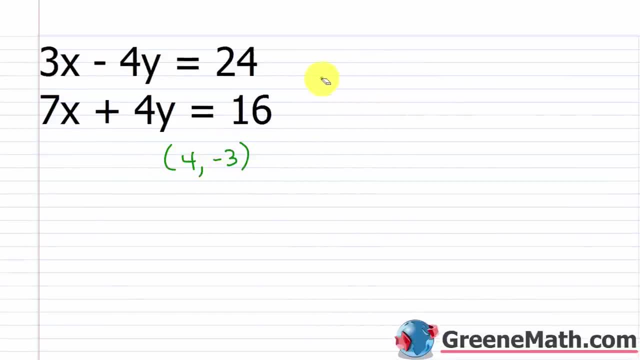 And again, let's go ahead and check it in the original equations. Make sure that we have the right answer. So 3 times 4 for x minus 4 times negative, 3 for y equals 24.. 3 times 4 is 12.. 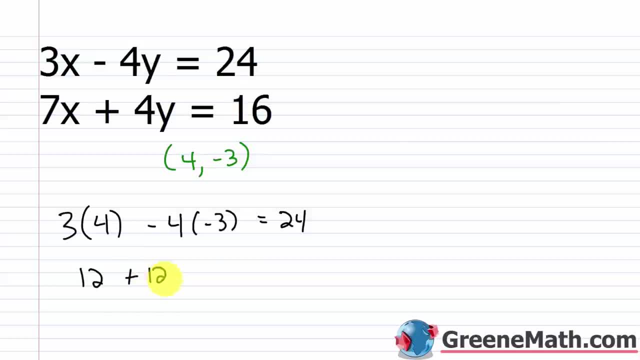 Negative 4 times negative. 3 is also 12.. So plus 12. This equals 24.. And it does Right: 12 plus 12 would be 24.. So that checks out, And then for the next equation we'd have 7.. 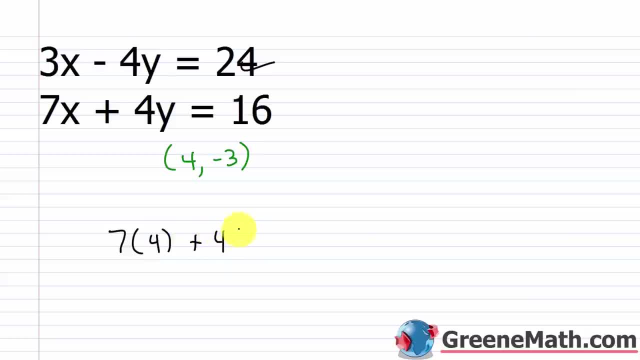 So 7 times plug in a 4 for x plus 4 times plug in a negative 3 for y, And this equals 16.. So 7 times 4 is 28 plus 4 times negative 3. That's negative 12.. 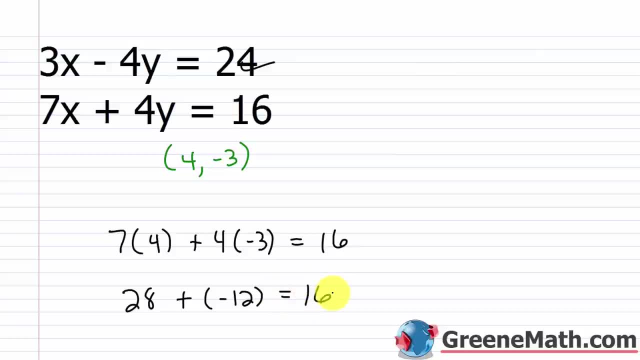 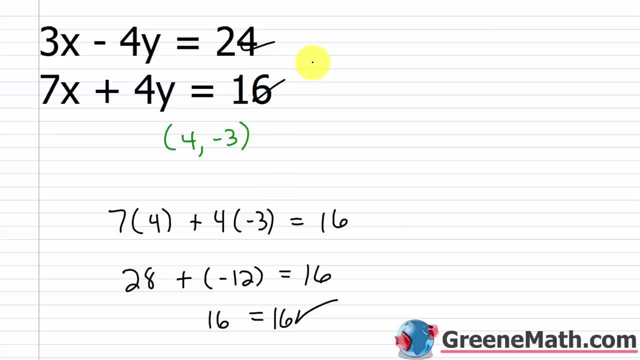 This equals 16.. And of course it does 28 minus 12 or 28 plus negative 12 is 16.. So you get 16 equals 16.. So yeah, that's true, 4 comma negative 3 is going to be the solution to this system. 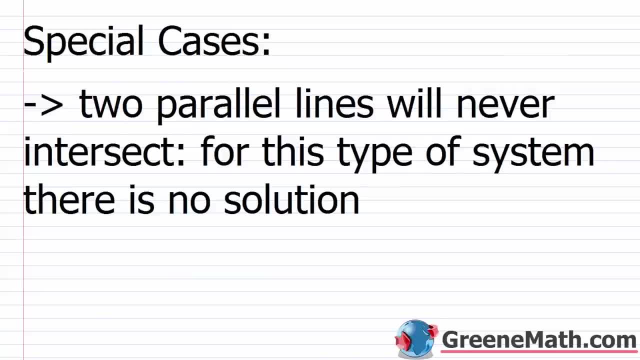 All right, So overall pretty easy. I feel like in the lesson we'll just do two examples. You could do more examples if you wanted to. We're going to do a practice set and some test exercises, but really not very difficult. 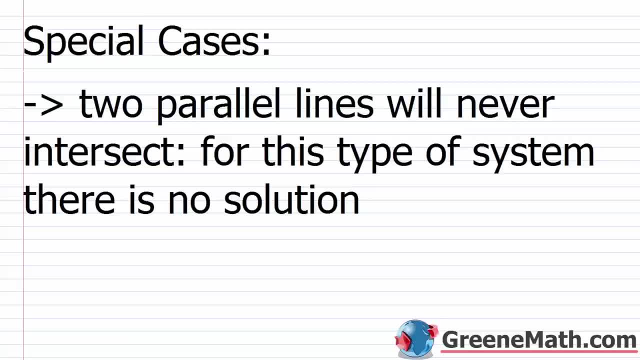 basically because I chose easy problems. If you had harder problems, you wouldn't even be able to find the solution from graphing because it would go off your coordinate plane. You know, if I had something with a solution, that was the ordered pair. 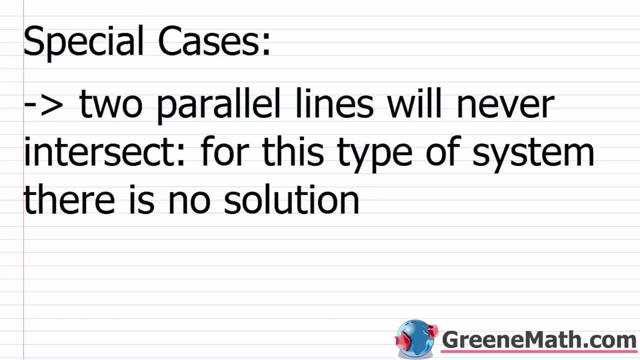 negative 3 eighths comma, I don't know, 2 tenths. You're not going to be able to graph that. Or if you had something that was like negative 150 comma 200, you're not going to be able to graph that. 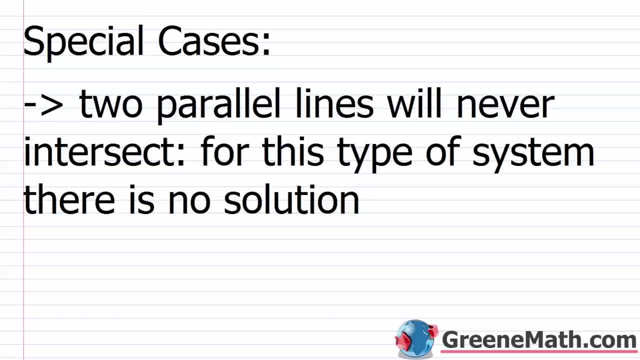 Okay, So you're going to be able to graph that. So you're going to be able to graph that. So now let's kind of move on and talk about special cases, And then in the next lesson we're going to go to a much more efficient way to do this. 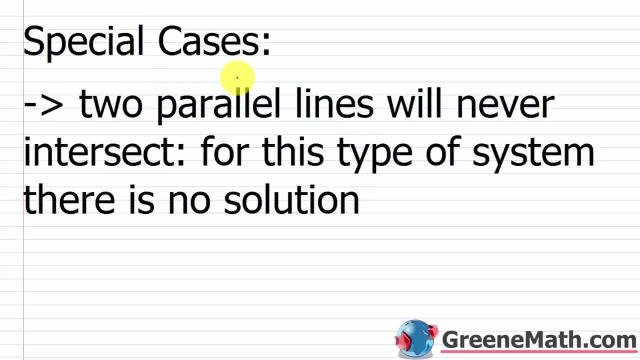 It's called substitution. So the special cases you're going to run across, You have systems that don't have a solution. So that occurs when you have two parallel lines, And two parallel lines, as you'll recall, will never intersect. So again, for this type of system, there is no solution. 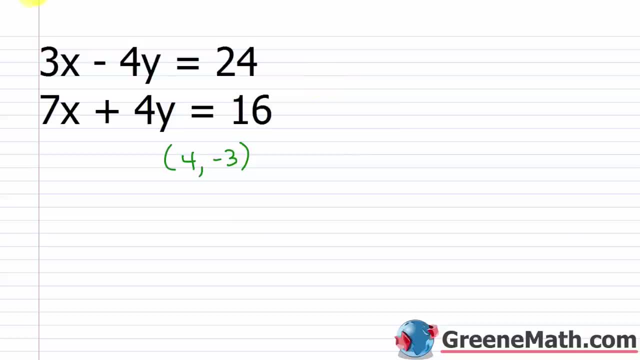 Again, let's go ahead and check it in the original equations. Make sure that we have the right answer. 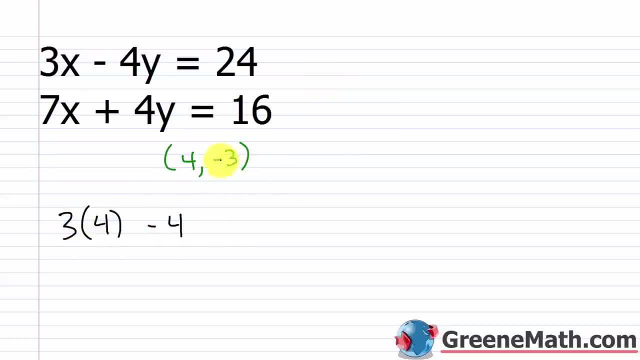 So 3 times 4 for x minus 4 times negative 3 for y equals 24. 3 times 4 is 12. Negative 4 times negative 3 is also 12. So plus 12. This equals 24, and it does, right? 12 plus 12 would not be true. 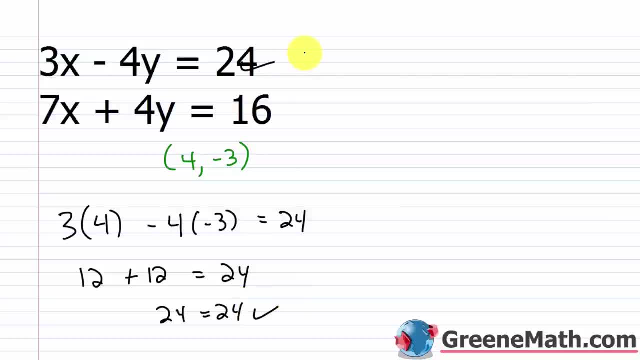 be 24. So that checks out. And then for the next equation, we'd have 7 times plug in a 4 for x plus 4 times plug in a negative 3 for y. And this equals 16. So 7 times 4 is 28 plus 4 times 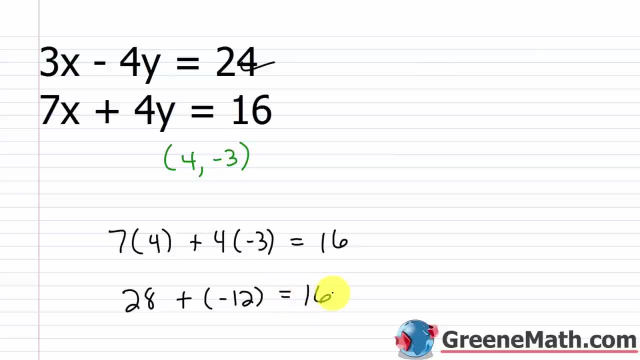 negative 3. That's negative 12. This equals 16. And of course it does. 28 minus 12 or 28 plus 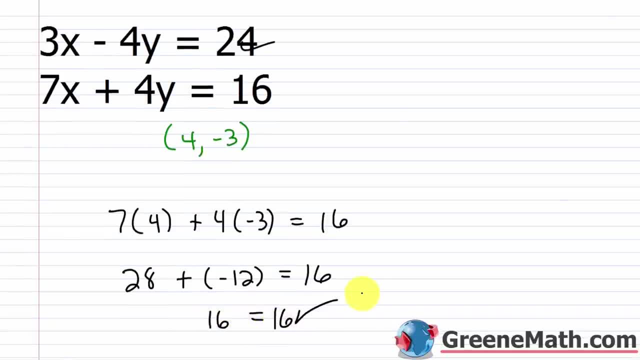 negative 12 is 16. So you get 16 equals 16. So yeah, that's true. 4 comma negative 3 is going 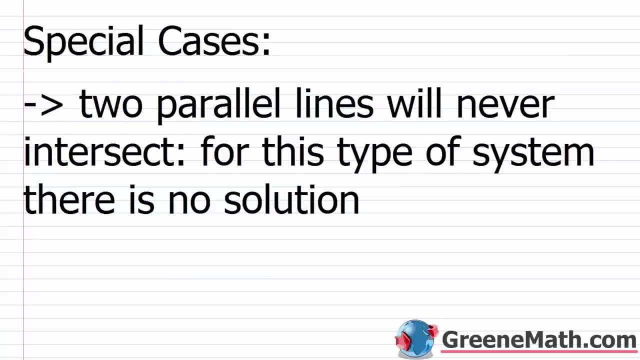 to be the solution to this system. All right. So overall, pretty easy. I feel like in the lesson, we'll just do two examples. You could do more examples if you wanted to. We're going to do a practice set and some test exercises, but really not very difficult, basically because I chose easy problems. If you had harder problems, you wouldn't even be able to find the solution from 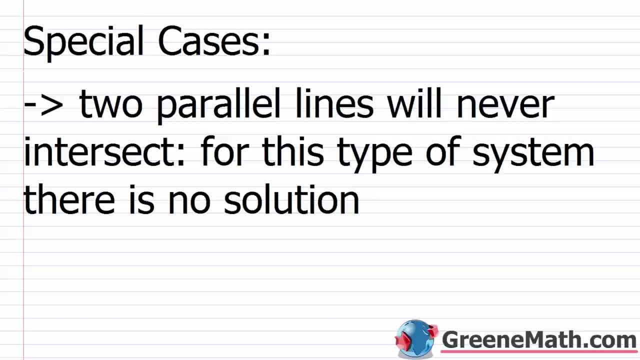 graphing because it would go off your coordinate plane. You know, if I had something with a solution that was the ordered pair, negative 3 eighths comma, I don't know, two tenths. You're 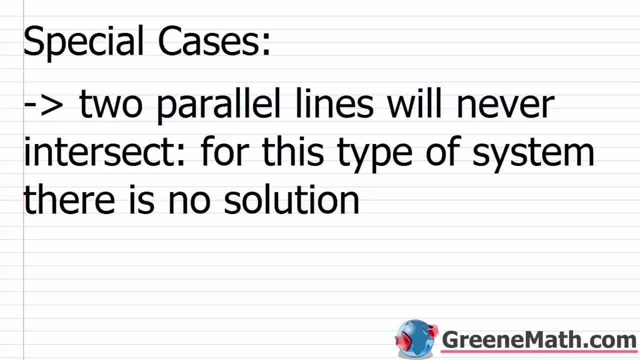 not going to be able to graph that. Or if you had something that was like negative 150 comma 200, you're not going to be able to graph that. Only with a computer. So now let's kind of move on 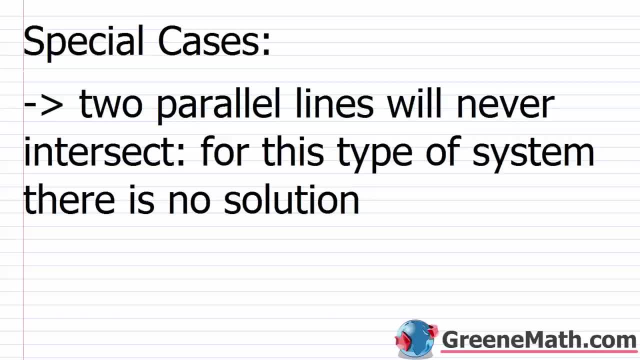 and talk about special cases. And then in the next lesson, we're going to go to a much more efficient way to do this. It's called substitution. So the special cases you're going to run across, you have systems that don't have a solution. So that occurs when you have two parallel lines. And two parallel lines, as you'll recall, will never intersect. So again, for this type of system, there is no solution. No solution. And you'll recall when we did our lessons on slope, we talked about parallel lines having the same slope or the same steepness. 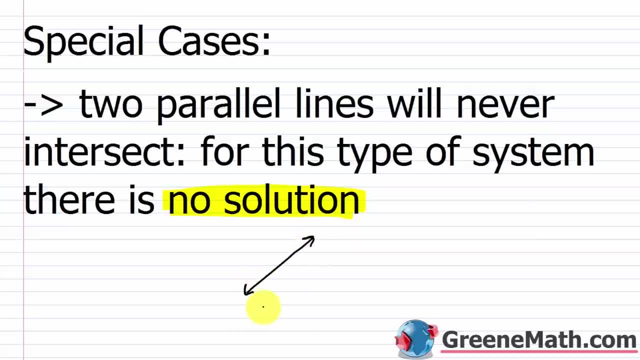 So they kind of look like this. So I know that's not perfect, but this would be an example where you just, you don't have a situation where you're ever going to intersect. 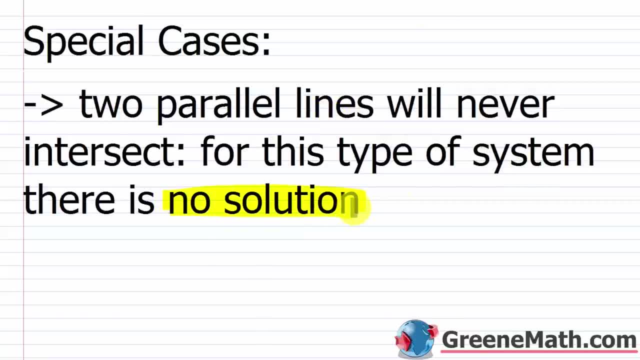 No solution And you'll recall, when we did our lessons on slope, we talked about parallel lines having the same slope or the same steepness, So they kind of look like this. So I know that's not perfect, but this would be an example. 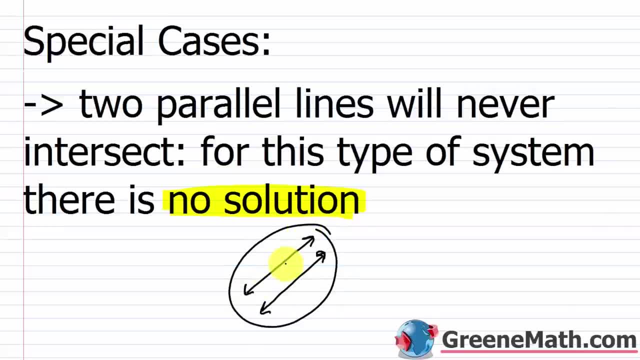 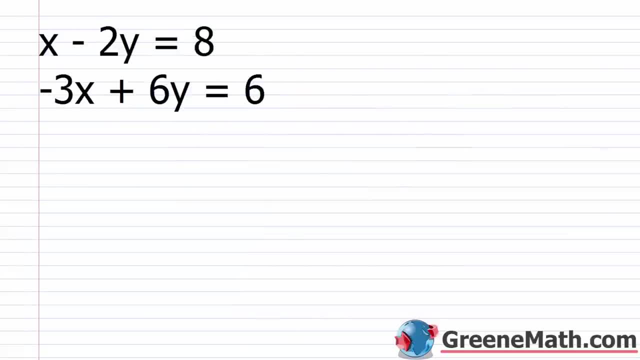 where you just you don't have a situation where you're ever going to intersect, So there's no solution because there's no ordered pair that lies on both lines. So here is an example of one where you won't get a solution. So x minus 2y equals 8, negative 3x plus 6y equals 6.. 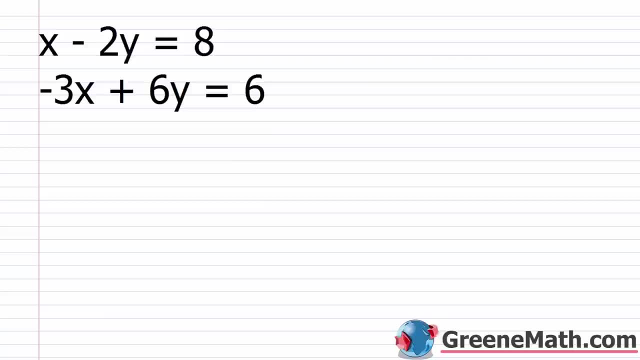 So let's go ahead and solve each for y And you're going to see right away, because they're in slope intercept form, that they're parallel lines. So I'm going to solve this for y, So we'll have negative 2y. 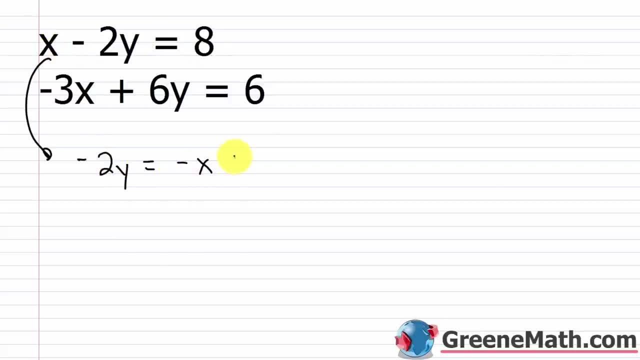 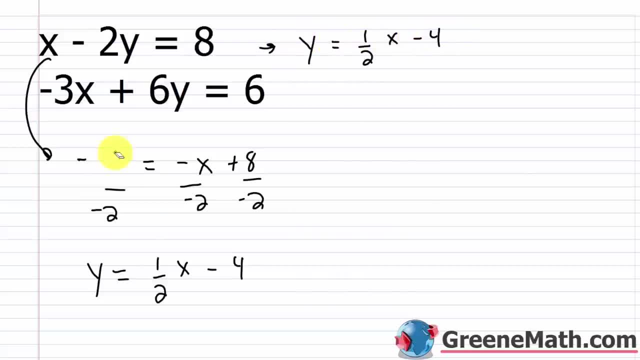 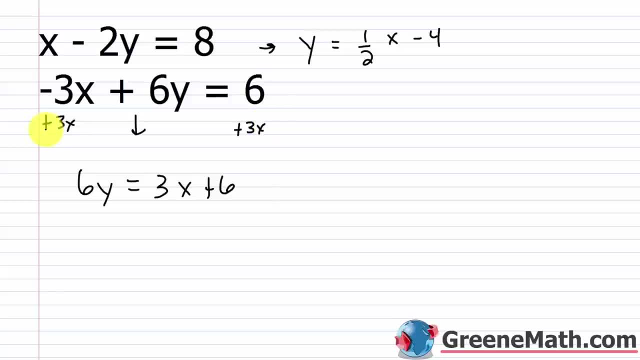 Again. I just added 3x to both sides. That's all I did. So that would cancel. 6y equals 3x, which is now over here, plus 6.. Okay, so now I would divide both sides by 6.. 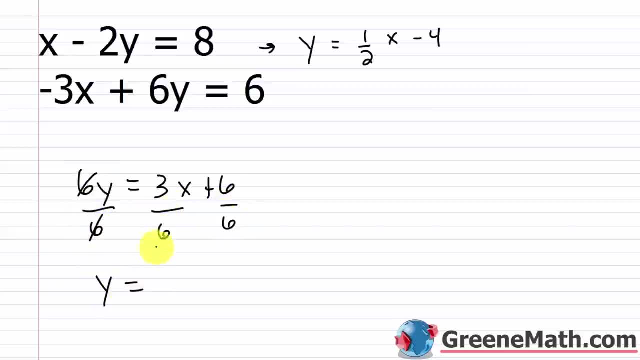 And this will cancel, You'll get: y is equal to 3 over. 6 is 1 half, So 1 half x plus 1.. So y equals 1 half x plus 1.. So immediately, what you can tell is that these two lines have the same slope right. 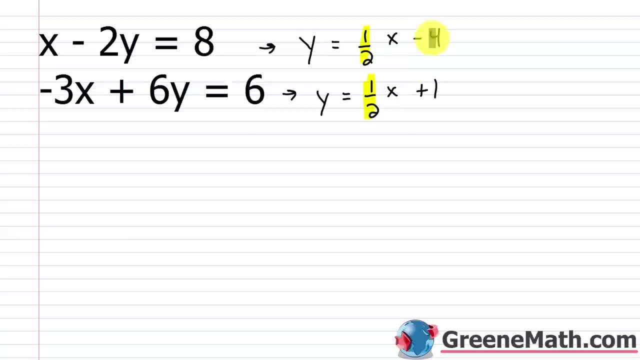 The coefficient for x in each case is 1 half. But different y intercepts. This y intercept would occur at 0 comma negative 4.. This one would occur at 0 comma 1.. So same slope, different y intercepts, parallel lines. 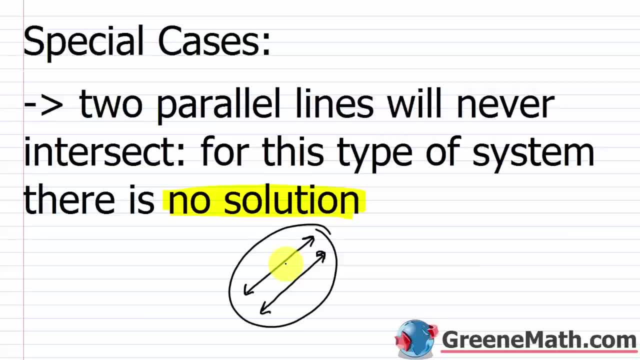 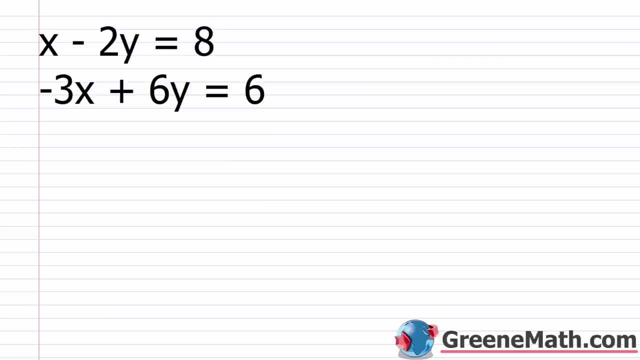 So there's no solution because there's no ordered pair that lies on both lines. So here is an example of one where you won't get a solution. So x minus 2y equals 8, negative 3x plus 6y equals 6. So let's go ahead and solve each for y. And you're going to see right away, because they're in slope intercept form, that they're parallel lines. So I'm going to solve this for y. So we'll have negative 2y. I'm just going to subtract x away from each side is equal to negative x plus 8, divide both sides by negative 2. You'll get y is equal to 1 half x minus 4. 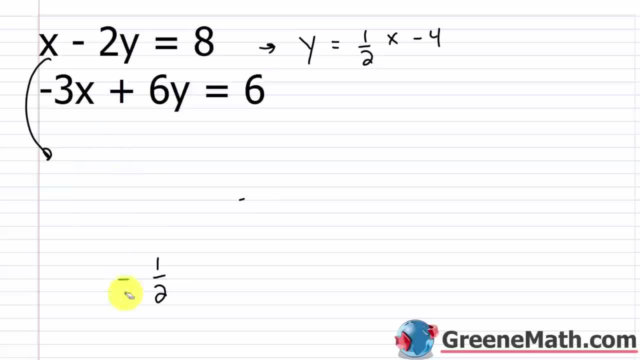 Okay, that's easy enough. And then let's go ahead and do the other one. So if I solve this for y, I'd add 3x to both sides. So I'd have 6y is equal to 3x plus 6. 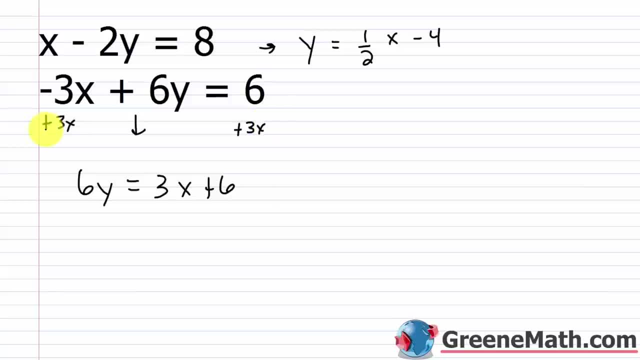 Again, I just added 3x to both sides. That's all I did. So that would be negative 2y. And then I'd add 3x to both sides. So I'd have 6y is equal to 3x plus 6. 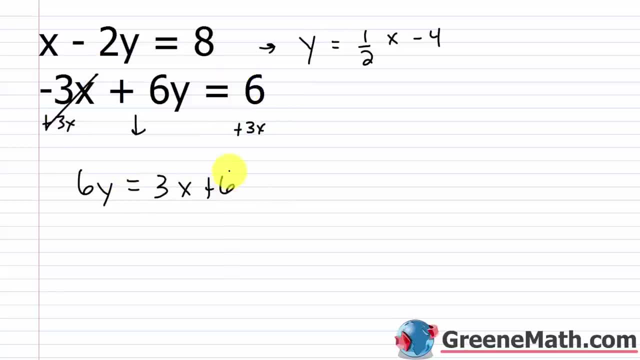 cancel 6y equals 3x which is now over here plus 6. Okay so now I would divide both sides by 6 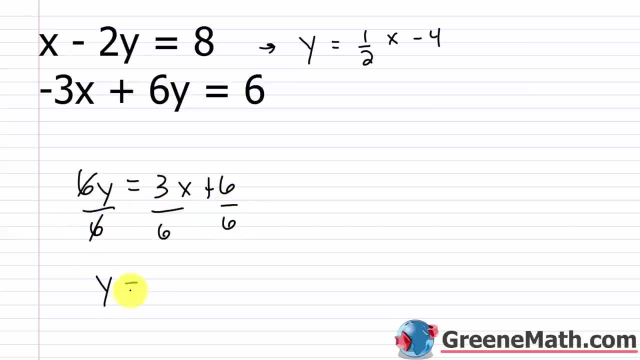 and this will cancel. You'll get y is equal to 3 over 6 is 1 half. So 1 half x plus 1. So y equals 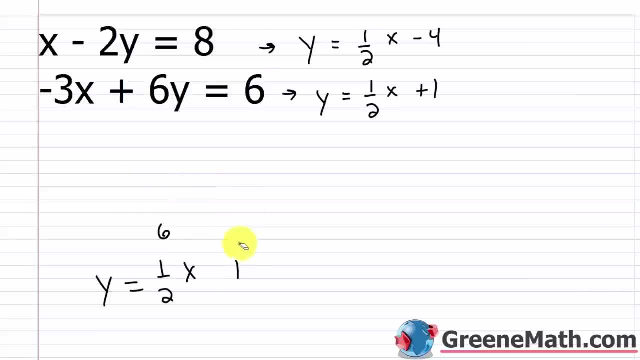 1 half x plus 1. So immediately what you can tell is that these two lines have the same slope. 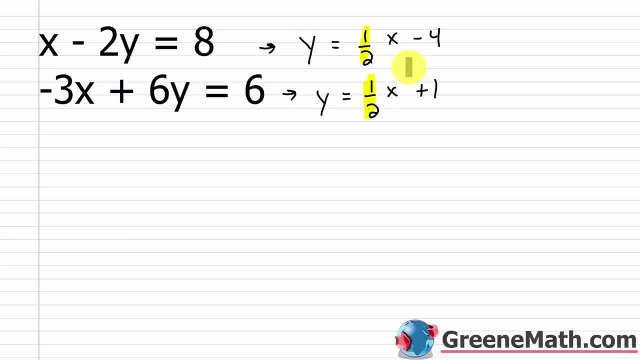 Right the coefficient for x in each case is 1 half but different y intercepts. This y intercept would occur at 0 comma negative 4. This one would occur at 0 comma 1. So same slope different y 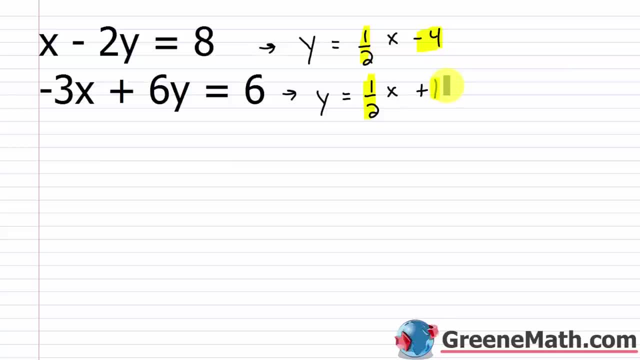 intercepts parallel lines they'll never intersect and so you don't have a solution. Now I'm going 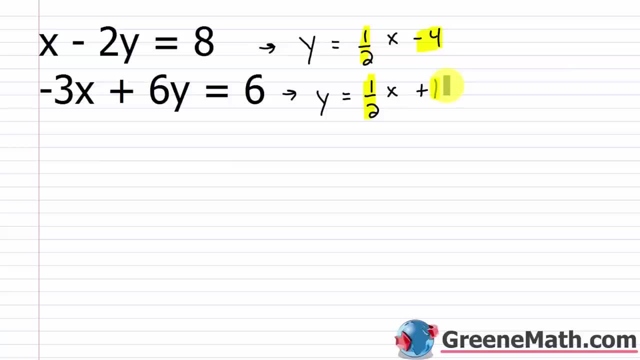 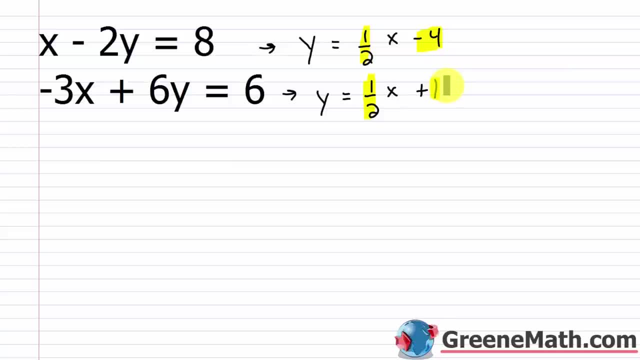 They'll never intersect, And so you don't have a solution. Now I'm gonna go ahead and graph this one, But when we get these in the future, you know we might graph them for completeness. But basically, if you got that on a test, 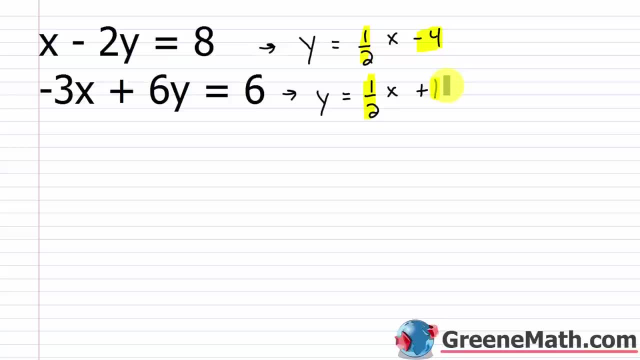 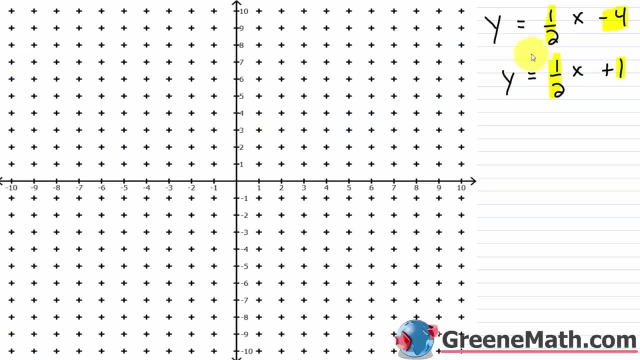 once you figure out that they're parallel lines, go ahead and just say okay, there's no solution, There's no solution and move on. All right. so for the first one to graph it, the y intercept is at 0 comma negative 4.. 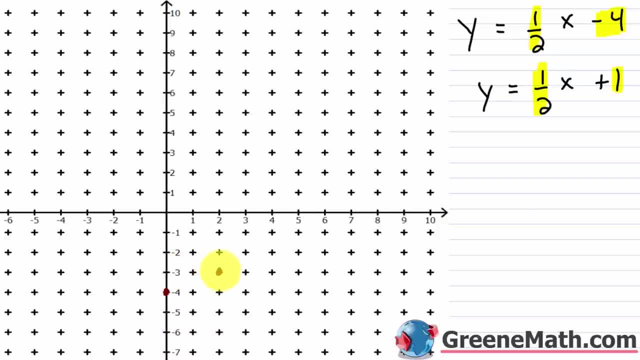 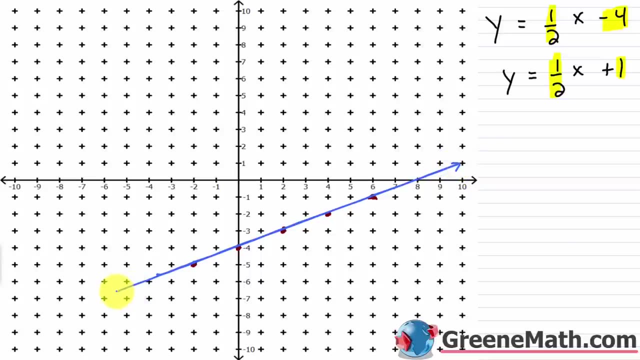 That's here And the slope is 1 half. So up, 1 over 2.. Up, 1 over 2.. Up, 1 over 2.. And I'll do down 1 to the left, 2.. All right, the next one has a y intercept. 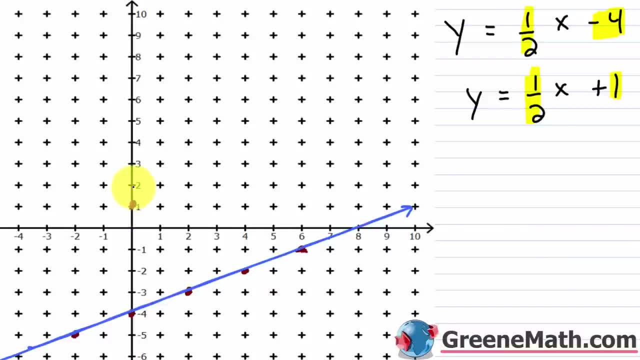 that occurs at 0 comma 1.. That's right here. And the slope again is 1 half. So up 1 over 2.. Up 1 over 2.. Up 1 over 2.. Or down 1 to the left, 2.. 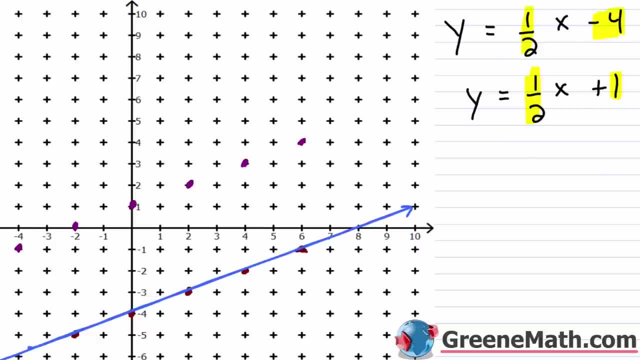 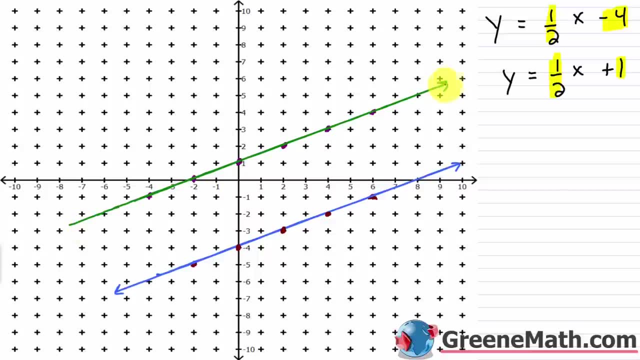 Down 1 over 2.. Down 1 to the left- 2.. So let's go ahead. Of course they're not perfectly drawn, But you can see that these would be parallel lines, So there would never be a solution for the system. 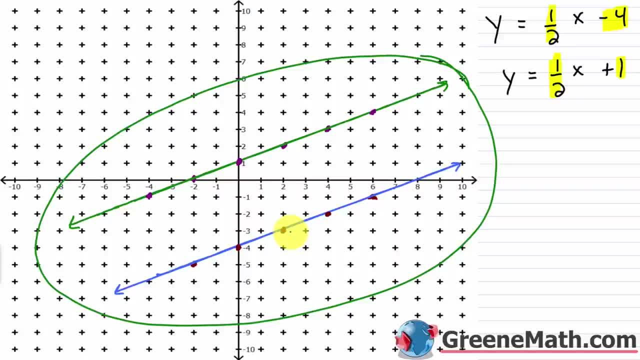 because these two lines would never intersect And therefore there's not an ordered pair that exists that would be on both of the lines. So there's never going to be a solution. So you see this And you put: no solution, No solution. 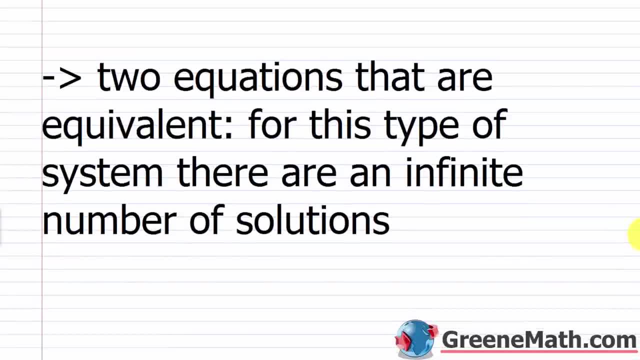 All right, so let's also talk about another scenario that you'll run across. Remember I said there were two special cases. The second case is you have two equations that are equivalent, So for this type of system, there are an infinite number of solutions. 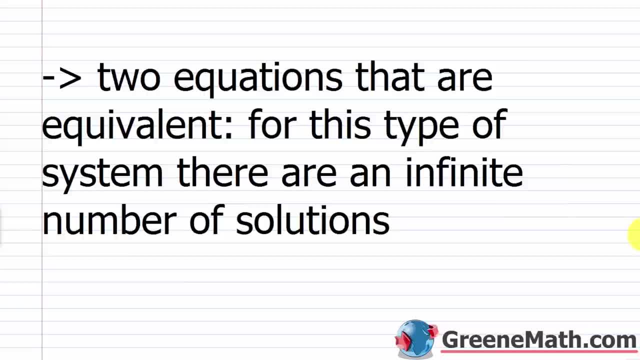 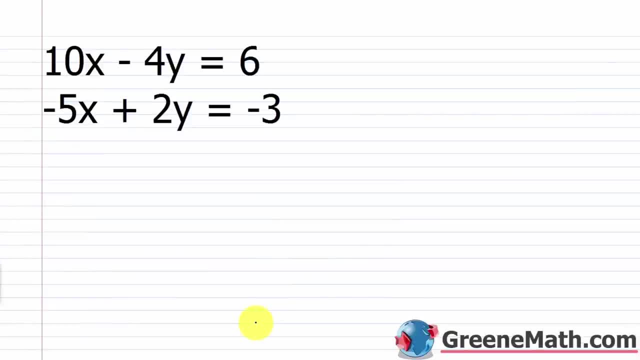 So essentially, what happens is you solve both of the equations for y And you end up seeing that they're the exact same equation. So here's an example of that: We have 10x minus 4y equals 6.. And we have negative 5x plus 2y equals negative 5x. 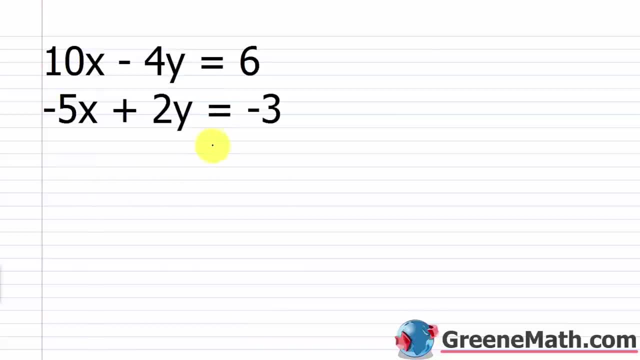 So this is the exact same equation, If you kind of look at it, and I multiply both sides of the equation by negative 2, here I would get this equation. So these equations are the same, They're just manipulated algebraically to look different. 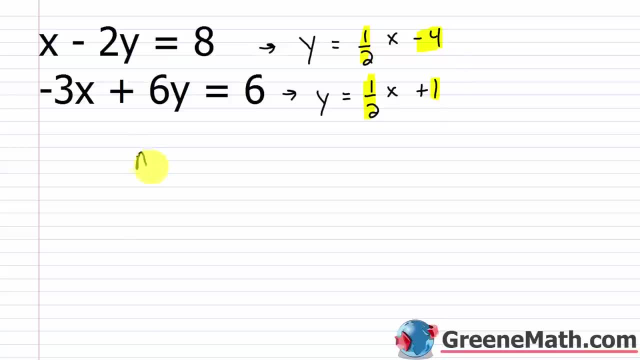 they're parallel lines go ahead and just say okay there's no solution there's no solution and move 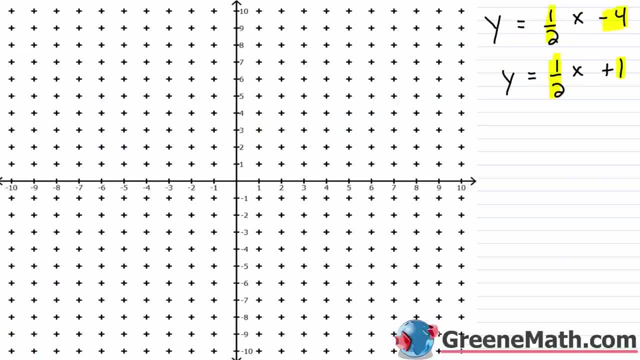 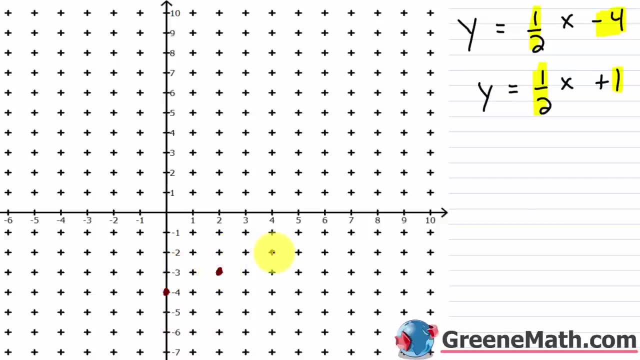 on. All right so for the first one to graph it the y intercept is at 0 comma negative 4 that's here and the slope is 1 half. So up 1 over 2 up 1 over 2 up 1 over 2 and I'll do down 1 to the left 2. 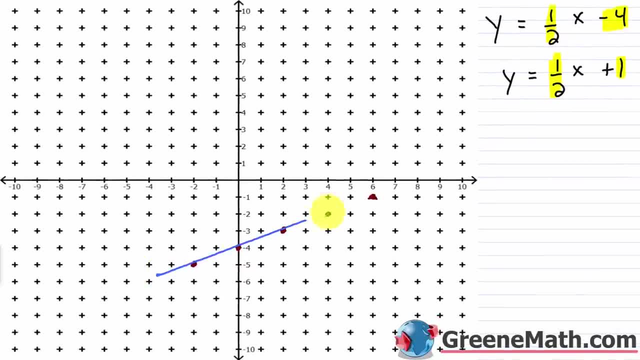 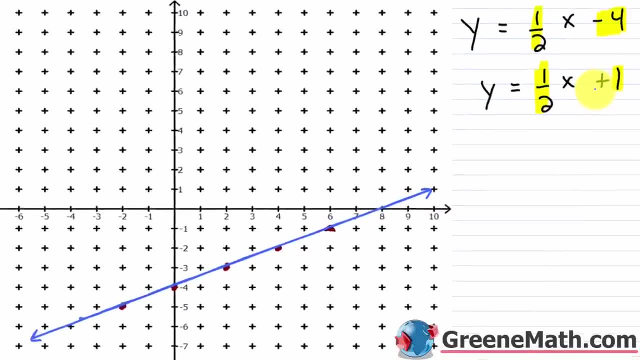 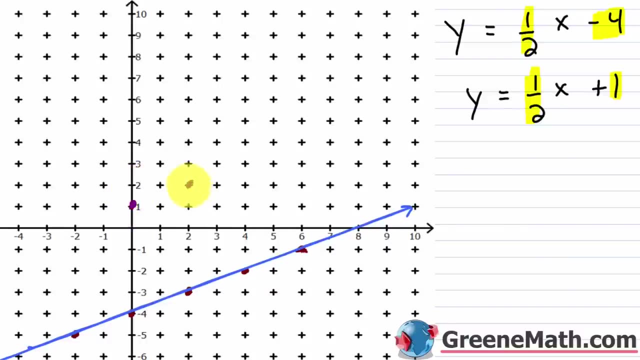 All right the next one has a y intercept that occurs at 0 comma 1 that's right here and the slope again is 1 half. So up 1 over 2 up 1 over 2 up 1 over 2 or down 1 to the left 2 down 1 to the left 2. So let's go ahead 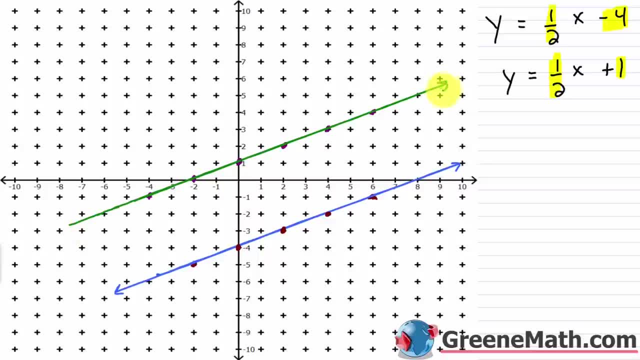 of course they're not perfectly drawn but you can see that these would be parallel lines so there would never be a solution for the system because these two lines would never intersect and therefore there's not an ordered pair that exists that would be on both of the lines so there's never going to be a solution. So you see this and you put no solution no solution. All right so let's 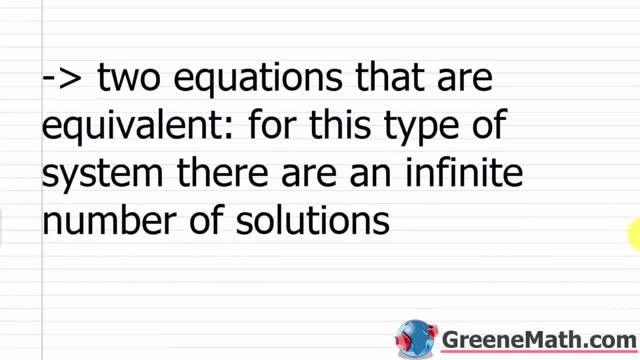 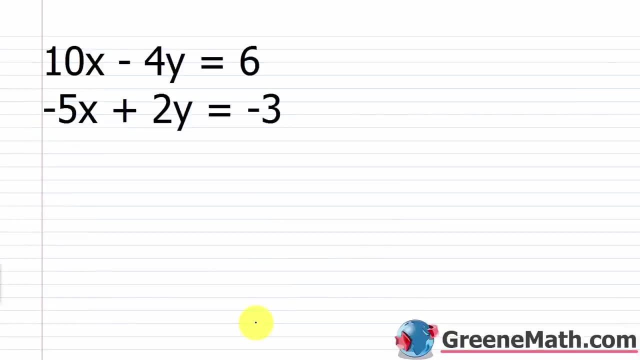 also talk about another scenario that you're running around with. So let's say you have a system where you have two equations that are equivalent so for this type of system there are an infinite number of solutions so essentially what happens is you solve both of the equations for y and you end up seeing that they're the exact same equation. So here's an example of that we have 10x minus 4y equals 6 we have negative 5x plus 2y equals negative 3. So this is the exact same equation if you kind of look at it and I multiply both sides of the equation by negative 2 here I would get this equation. So these equations are the same they're just 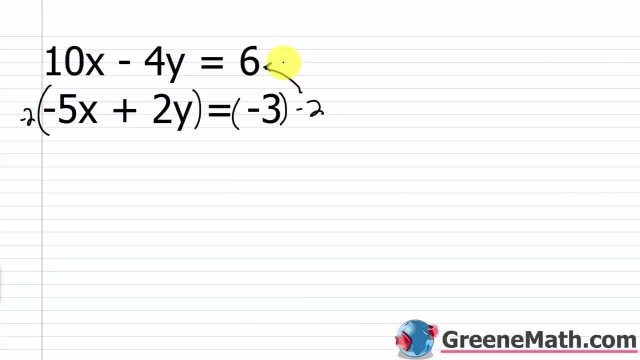 manipulated algebraically to look different and so you're going to see an example of this on your 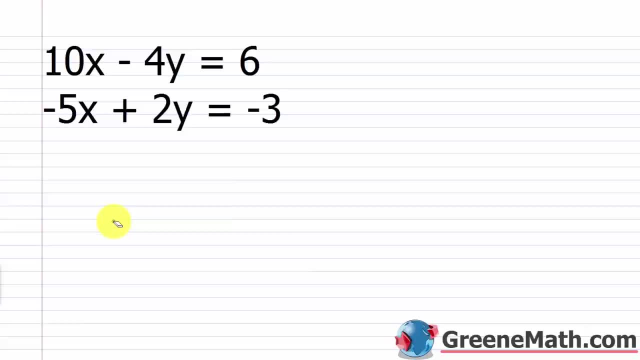 test or your homework and so if you see that and you spot it right away you can just say that there's an infinite number of solutions. But let's go through another process kind of the quicker way to do it if you don't spot it right away is just to solve each for y put it in slope intercept form I have 10x minus 4y equals 6 I would subtract 10x away from each side 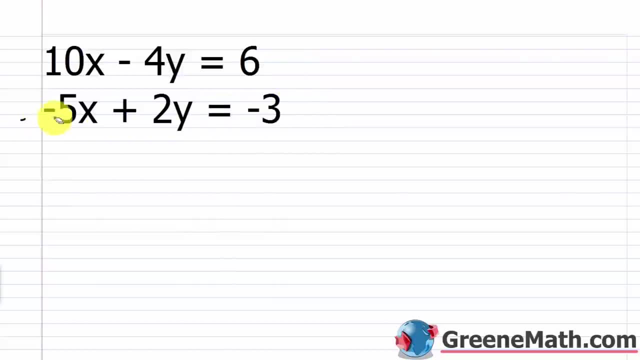 And so you're going to see an example of this on your test or your homework, And so if you see that and you spot it right away, you can just say that there's an infinite number of solutions. But let's go through another process, kind of a quicker way. 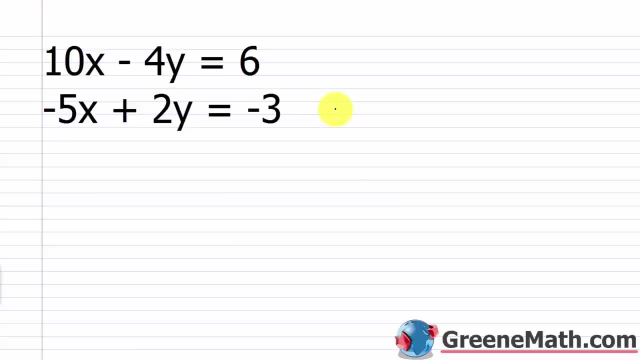 to do it. if you don't spot it right away, It's just to solve each for y. Put it in slope-intercept form and you'll see you have the same equation. So if I solve this guy for y, I have 10x minus 4y equals 6.. 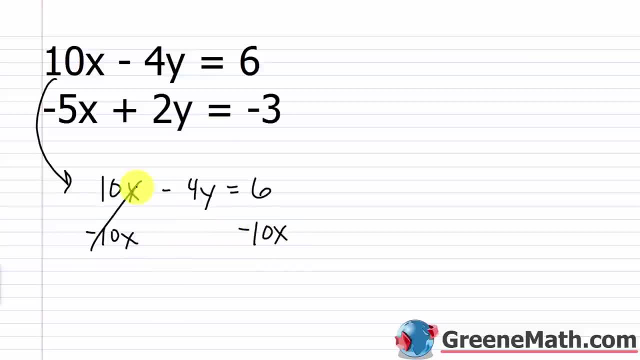 I would subtract 10x away from each side. That's going to cancel. I'll have negative 4y is equal to negative 10x. I'll have negative 4y is equal to negative 10x plus 6.. And I want to divide each side by 2.. 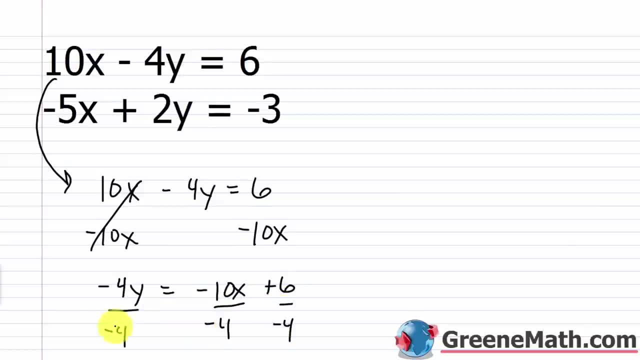 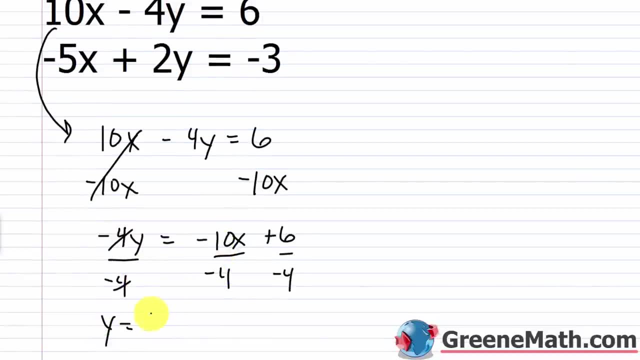 I'm going to divide by negative 4. now That's gone, And so I'll have: y is equal to negative. 10 over negative, 4 is 5. halves Negative over negative is positive. 10 divided by 2 is 5.. 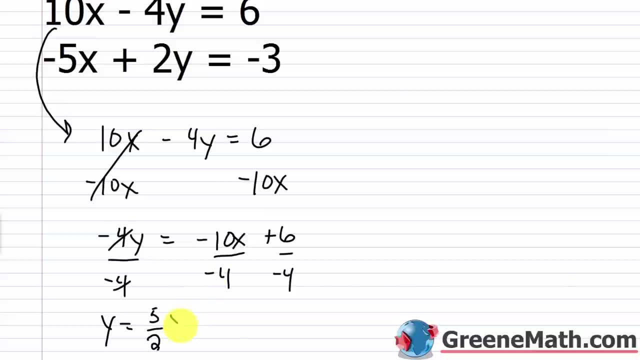 4 divided by 2 is 2.. So 5 halves. then times x, And then positive over negative is negative, 6 over 4, we could think of as 3 halves, Because 6 divided by 2 is 3.. 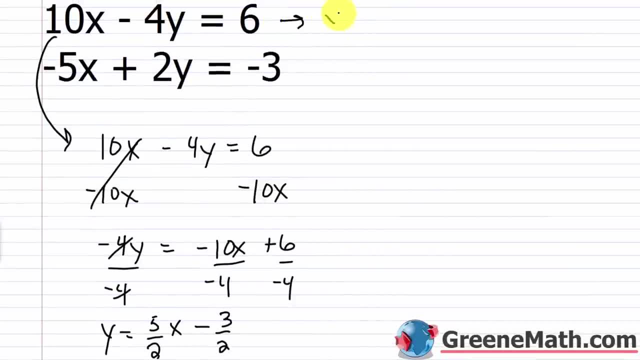 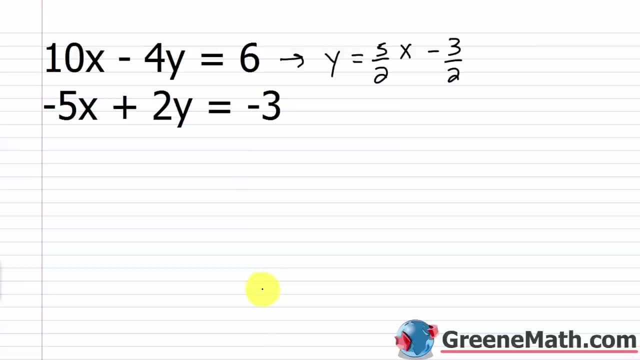 4 divided by 2 is 2.. So this one right here is: y equals 5 halves x minus 3 halves. Now the next one. when we solve it for y, we're going to see we get the exact same thing. 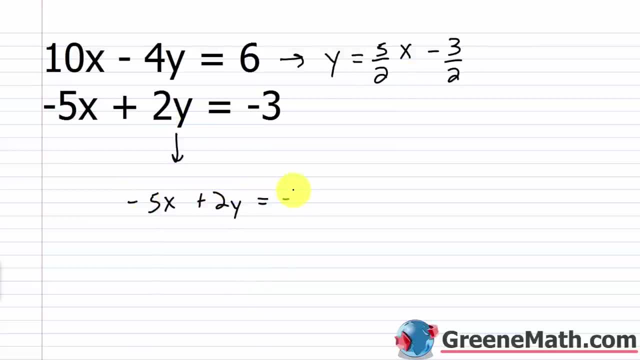 So again, negative. 5x plus 2y equals negative 3. Add 5x to each side of the equation. That's gone You'll have. 2y is equal to 5x minus 3.. Divide both sides of the equation by 2.. 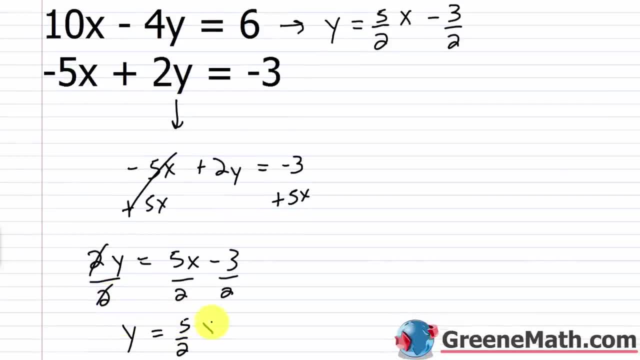 That's going to cancel. You'll have y equals 5 halves x minus 3 halves. So again, y equals 5 halves x minus 3 halves. Once you see that you have the exact same equation, you just stop and say: okay, the 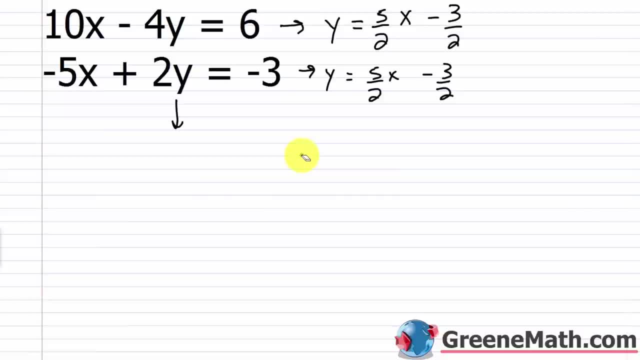 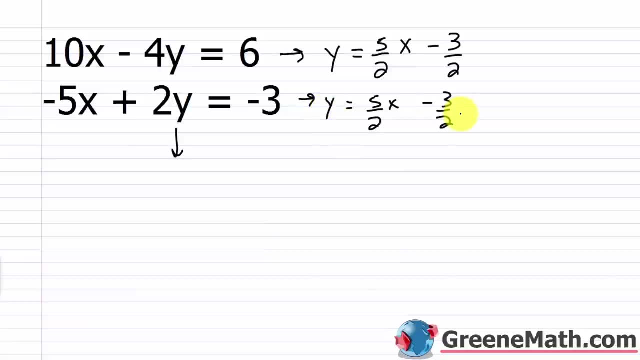 system contains the exact same equation. So there's an infinite number of solutions because whatever I plug in that works in this equation obviously works in this equation because they're the same equation. So there's an infinite number of solutions because a linear equation of two variables. 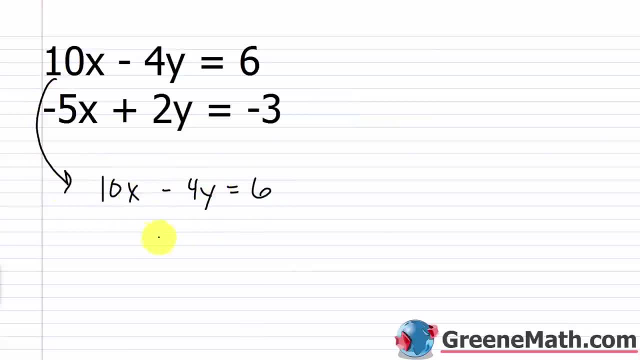 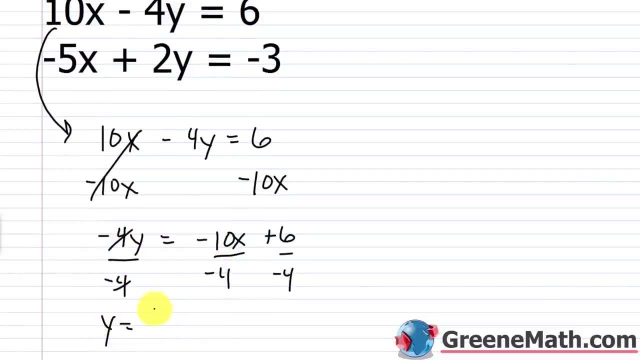 that's going to cancel I'll have negative 4y is equal to negative 10x I'll have negative 4y is equal to negative 10x plus 6 and I want to divide each side by negative 4 now that's gone and so I'll have y is equal to negative 4y is equal to negative 4y is equal to 10 over negative 4 is 5 halves right negative over negative is positive 10 divided by 2 is 5 4 divided by 2 is 2 so 5 halves then times x and then positive over negative is negative 6 over 4 we can think of as 3 halves right because 6 divided by 2 is 3 4 divided by 2 is 2 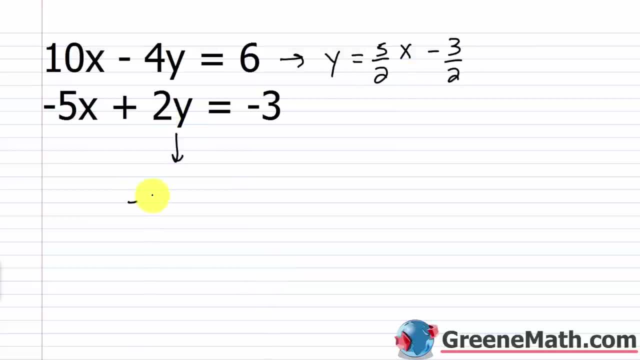 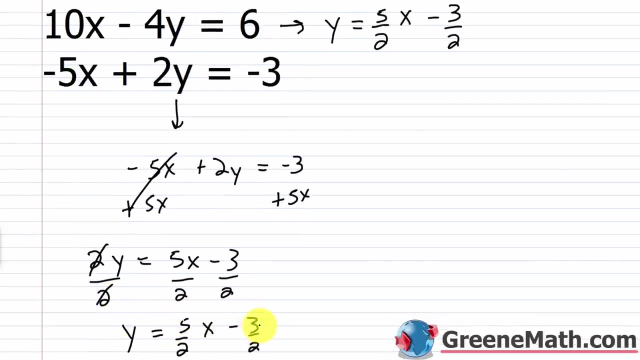 for y we're going to see we get the exact same thing so again negative 5x plus 2y equals negative 3 add 5x to each side of the equation that's gone you'll have 2y is equal to 5x minus 3 divide both sides of the equation by 2 that's going to cancel you'll have y equals 5 halves x minus 3 halves so again y equals 5 halves x minus 3 halves 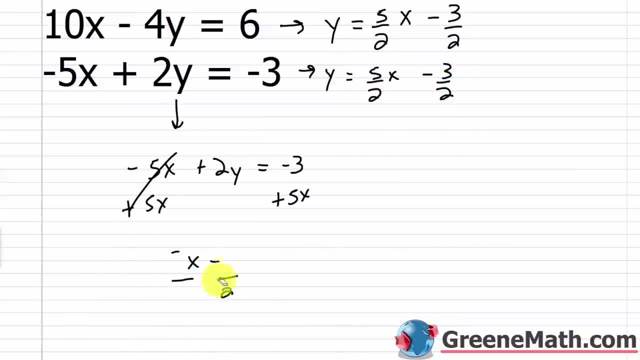 we're going to see we're going to get the exact same thing so again negative 5x plus 2y Once you see that you have the exact same equation, you just stop and say, okay, the system contains the exact same equation. 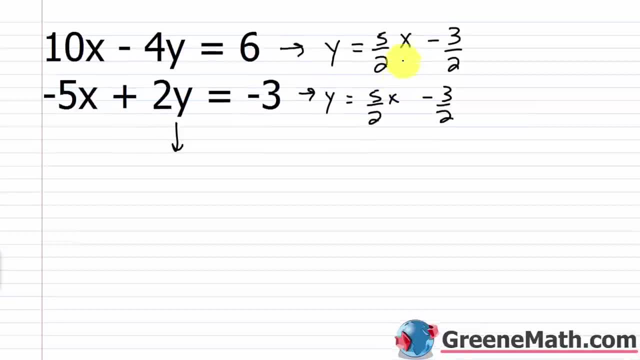 So there's an infinite number of solutions because whatever I plug in that works in this equation, obviously works in this equation because they're the same equation. 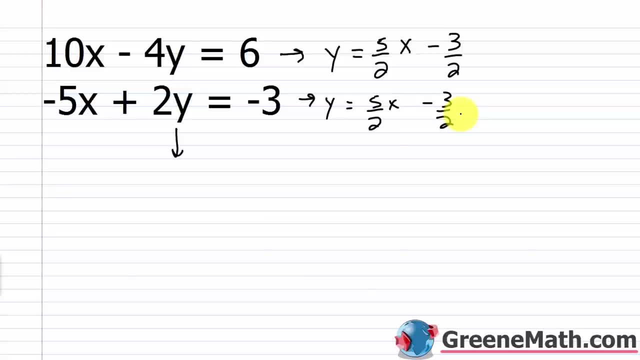 So there's an infinite number of solutions because a linear equation of two variables is gonna have an infinite number of solutions. 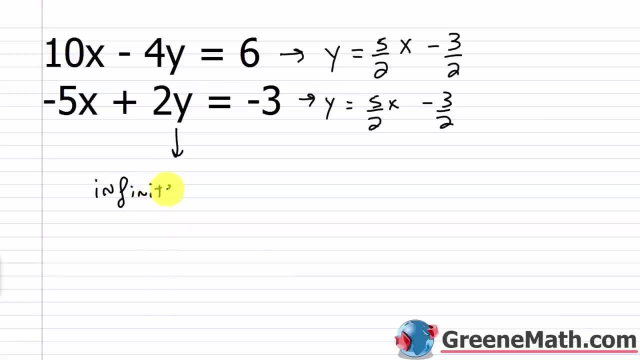 So there's an infinite number of solutions. 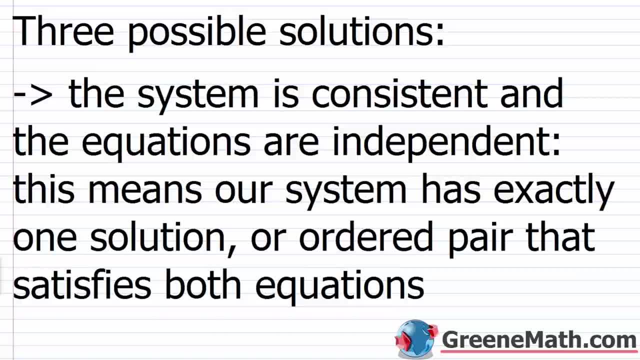 All right, so let's wrap up our lesson now. Just talk about there's three possible solutions. 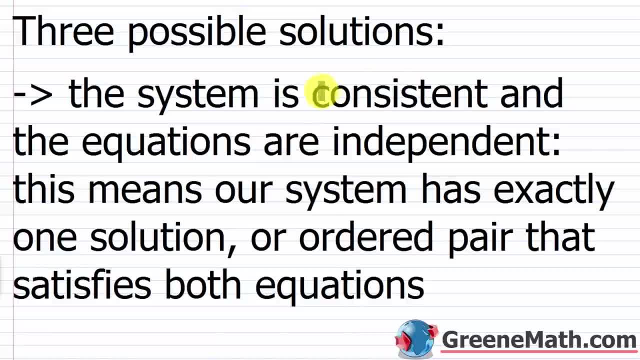 So the system is called consistent. The system is consistent and the equations are independent. Okay, so you're gonna hear that in your class. So this means our system has exactly one solution or one ordered pair that satisfies both equations. 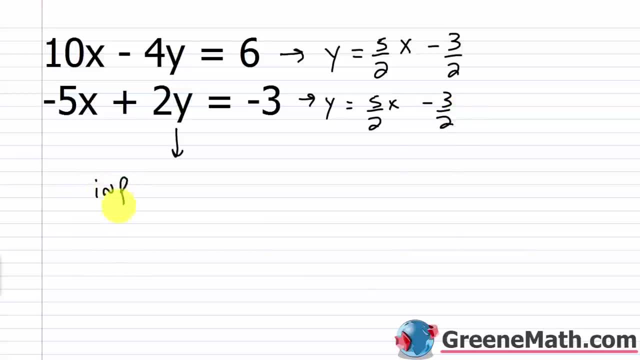 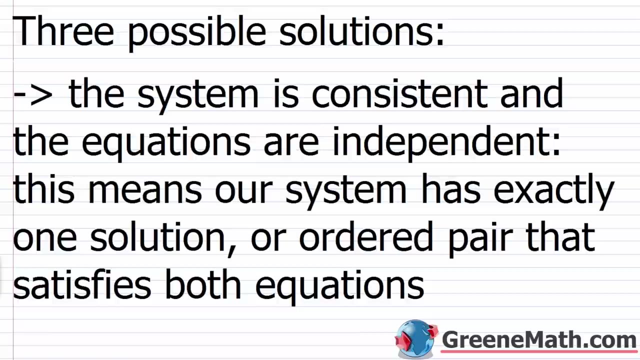 is going to have an infinite number of solutions. So there's an infinite number of solutions, All right. so let's wrap up our lesson now and just talk about there's three possible solutions. So the system is called consistent. The system is consistent and the equations are independent. okay, 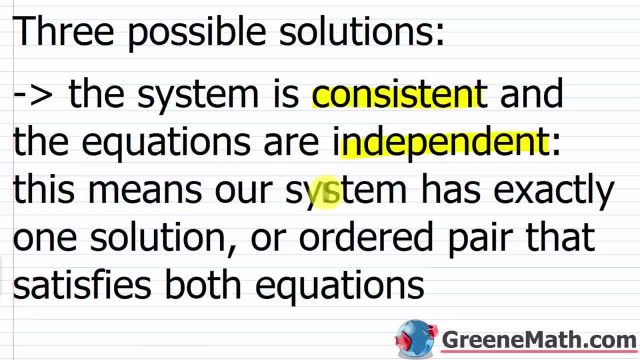 So you're going to hear that in your class. So this means our system has exactly one solution or one ordered pair, So we're going to have: Okay, good pair that satisfies both equations. So again, when this occurs- and this is 95% of the time- 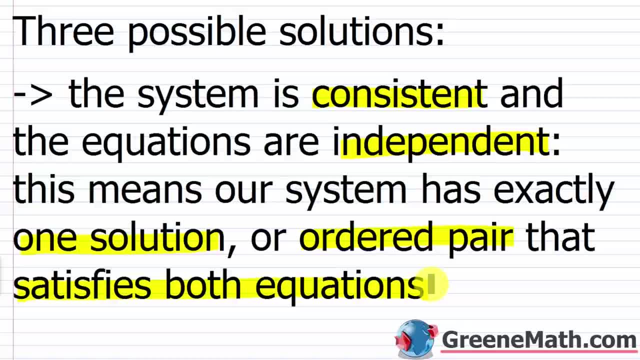 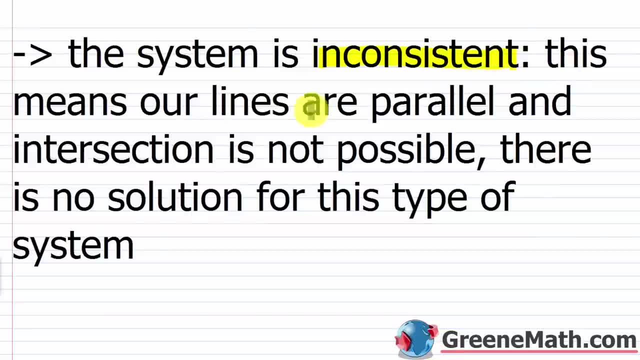 your system is consistent and the equations are independent. So that's most of the problems you're going to see. Now again, you're going to get special cases. So the system is inconsistent and this means that our lines are parallel, So they throw those at you every once in a while. 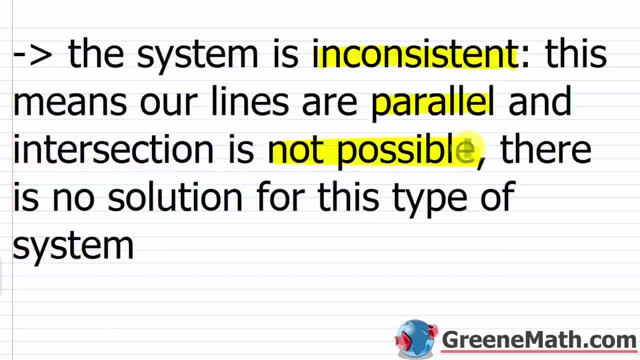 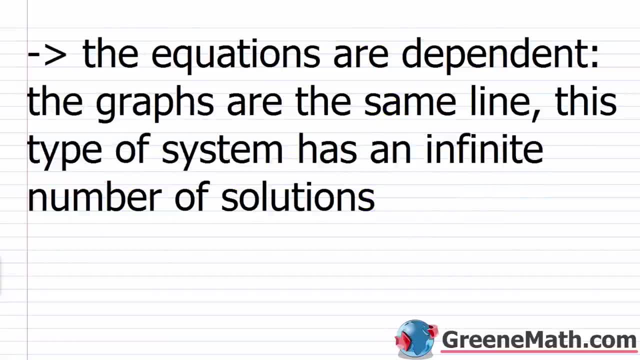 So an intersection is not possible, right? Parallel lines do not ever cross, So there is no solution for this type of system. All right, then the final type of system we have, that the equations are dependent, So the graphs are the same line. So we just saw that in the previous. 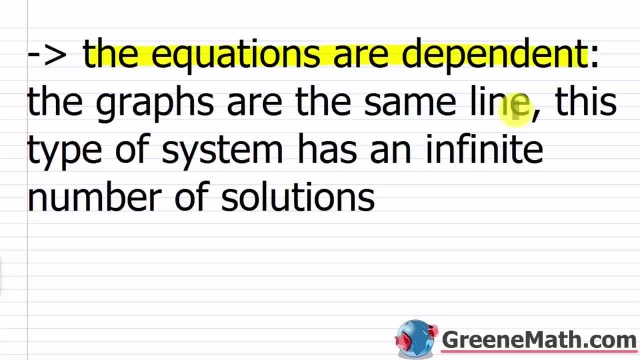 problem right. We solved each for y. we saw we have the exact same equation, So this type of system has an infinite number of solutions And again, the reason for that is it's the same equation And so if that equation by itself has an infinite number of solutions and anything that 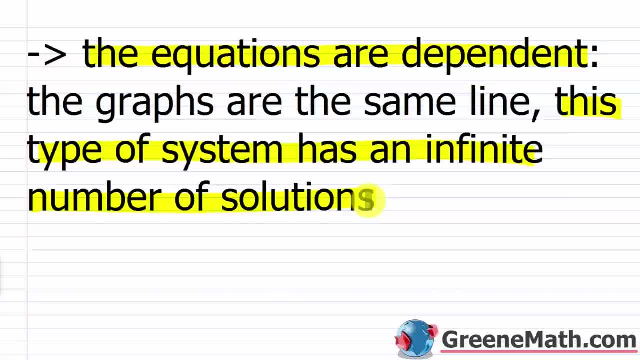 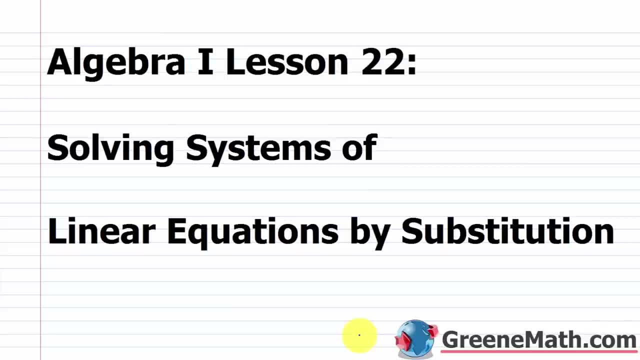 works in the first equation, obviously it's going to be the same equation. So if that equation by works in the second one, because they're the same right, so then the system has an infinite number of solutions. Hello and welcome to algebra one, lesson 22.. In this video we're going to learn 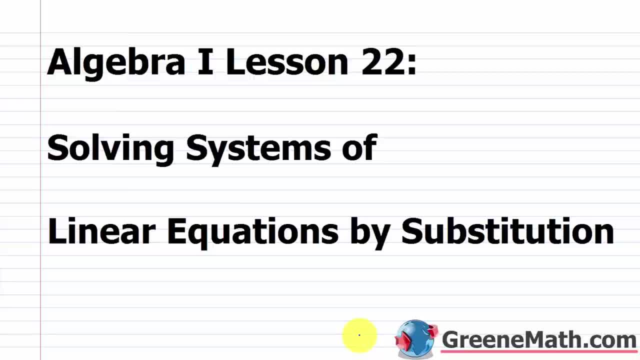 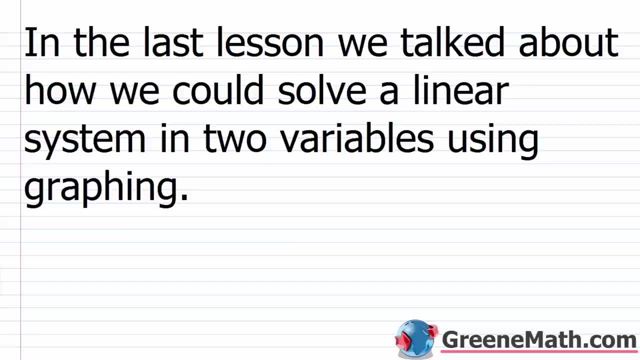 about solving systems of linear equations by substitution. So in the last lesson we talked about how we could solve a linear system in two variables using graphing, And what we found was, at the point of intersection we had an ordered pair that was on both lines. So therefore, 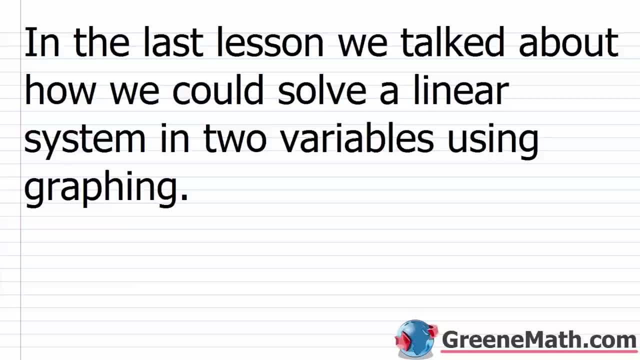 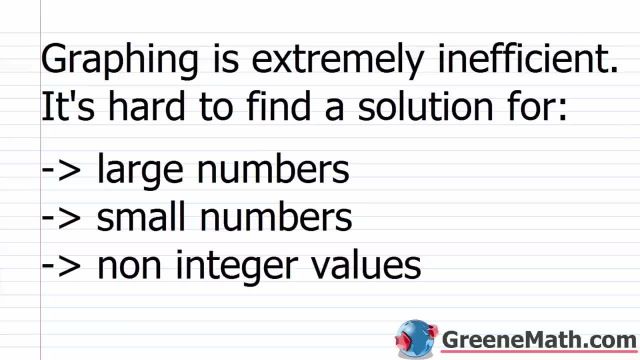 it was a solution to both equations of the system and it was a solution for our system. But there's some big problems with graphing. graphing is extremely inefficient And it's extremely hard to find a solution for we have large numbers, small numbers and non integer values, So in other words, 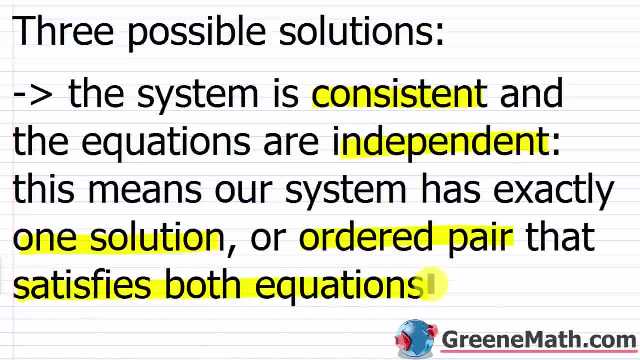 So again, when this occurs and this is 95% of the time, your system is consistent and the equations are independent. So that's most of the problems you're gonna see. 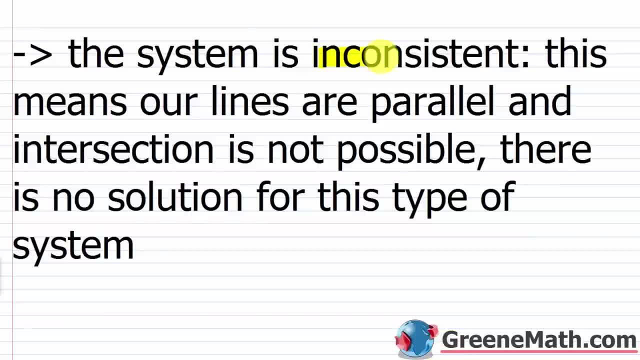 Now again, you're gonna get special cases. So the system is inconsistent and this means that our lines are parallel. So they throw those at you every once in a while. So an intersection is not possible, right? Parallel lines do not ever cross. 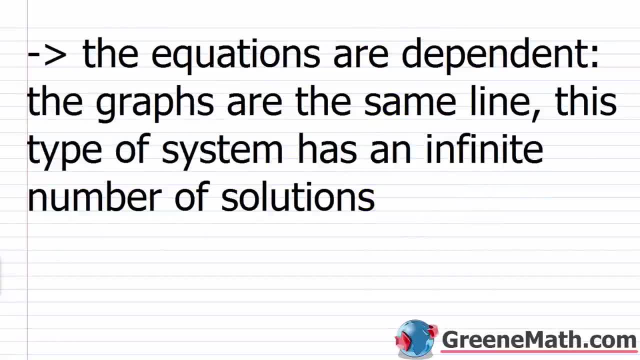 So there is no solution for this type of system. 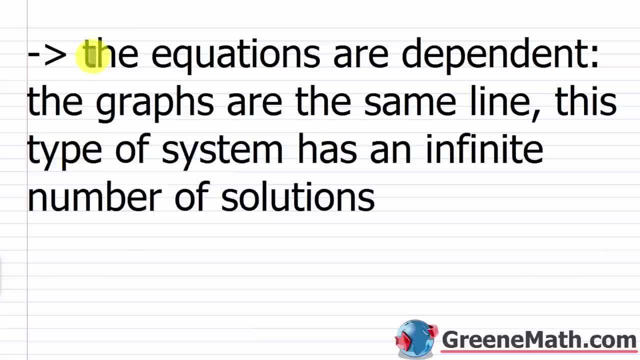 All right, then the final type of system, we have that the equations are dependent. So the graphs are the same line. So we just saw that in the previous problem, right? We solved each for y. We saw we had the exact same equation. 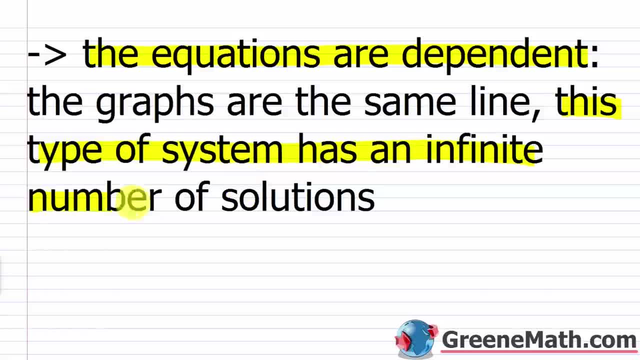 So this type of system has an infinite number of solutions. And again, the reason for that is it's the same equation. 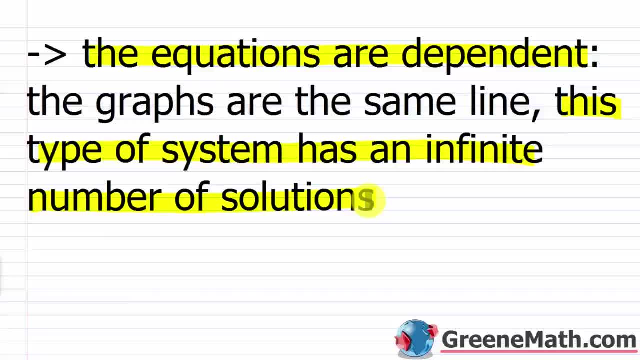 And so if that equation by itself has an infinite number of solutions and anything that works in the first equation obviously works in the second one because they're the same, right? So then the system has an infinite number of solutions. 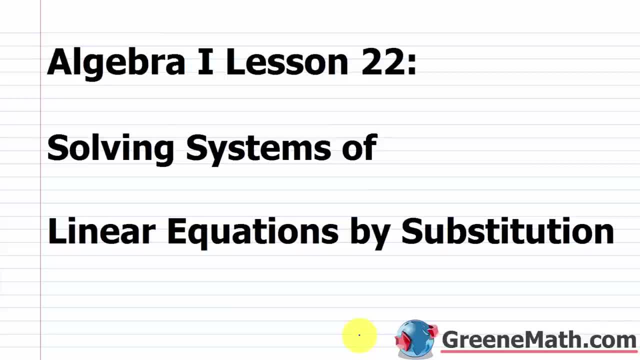 Hello and welcome to Algebra 1 Lesson 22. In this video, we're gonna learn about solving systems of linear equations by substitution. 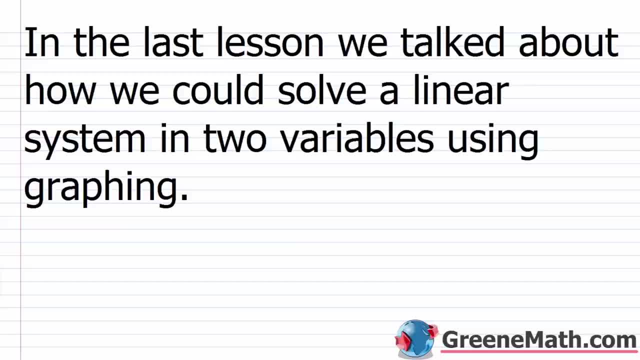 So in the last lesson, we talked about how we could solve a linear system in two variables using graphing. And what we found was at the point of intersection, we had an ordered pair that was on both lines. So therefore it was a solution to both equations of the system and it was a solution for our system. But there's some big problems with graphing. 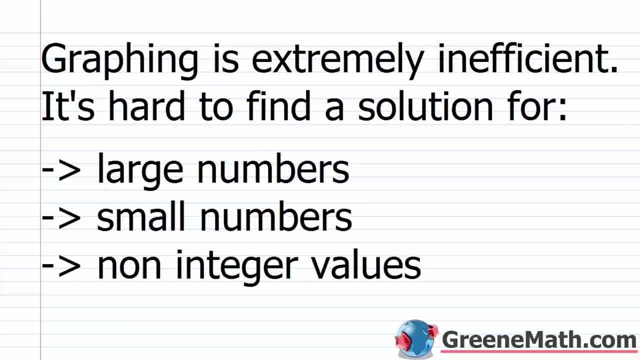 Graphing is extremely inefficient and it's extremely hard to find a solution for we have large numbers, small numbers, and non-integer values. 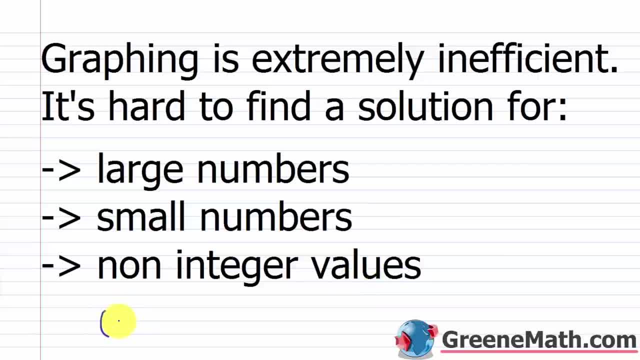 So in other words, if the solution was something like negative 3 4ths comma 1 7th, something like that. 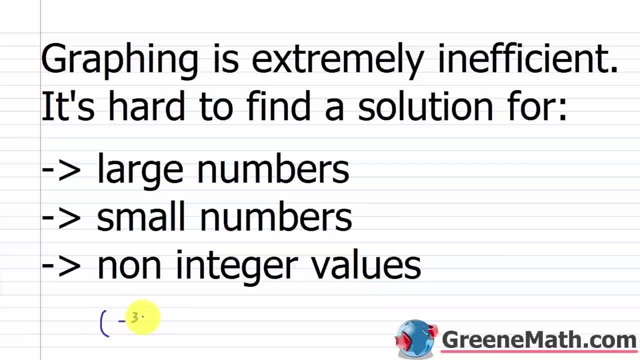 if the solution was something like negative: three fourths comma one, seventh, something like that. it's very hard to graph that. I know you can use a graphing calculator or computer program, But using a sheet of paper, like most of you are going to do on a test, it's not very efficient or very. 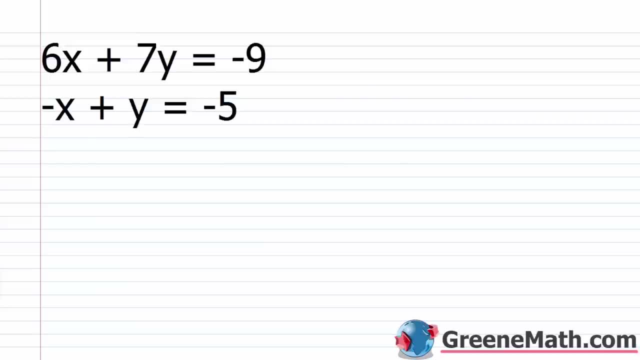 effective at all. So kind of the next thing we do is turn to an algebraic method. we got the concept down, we understand about a system of linear equations and what the solution means, But we need another way to kind of attack this type of problem. So with substitution I'm basically going 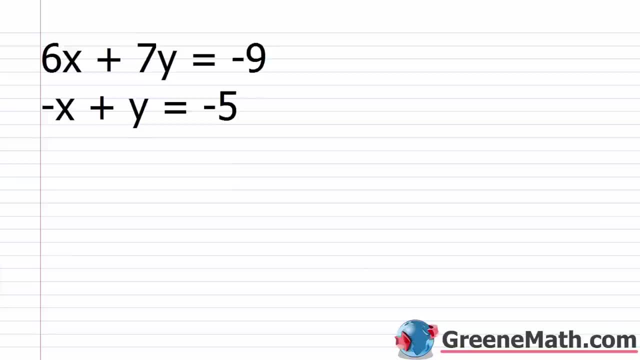 to substitute in for one of the variables and create a linear equation and one variable. So let me kind of go deeper into that. Let's say I have this problem: 6x plus 7y equals negative nine and negative x plus y equals negative five. What I can do is I can solve one of the equations. 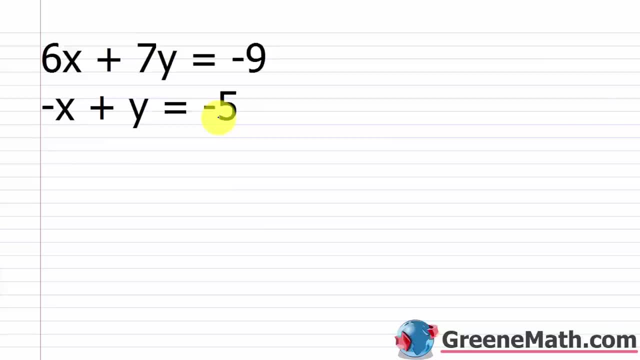 for one of the variables. Now, it doesn't matter which variable you pick And it doesn't matter which equation you start out with, But it's generally going to be easier if you look for a variable that has a coefficient of one. that's the easiest or the second easiest would be negative. 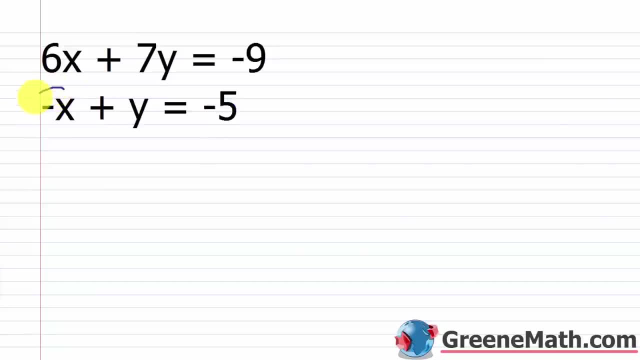 one. If I look at this equation, I'm going to have a coefficient of one and I'm going to have a coefficient of x. And if I look at this equation here, what I see is that I have a coefficient on the y variable of one. I have a coefficient on the x variable of negative one, So I can use either of. 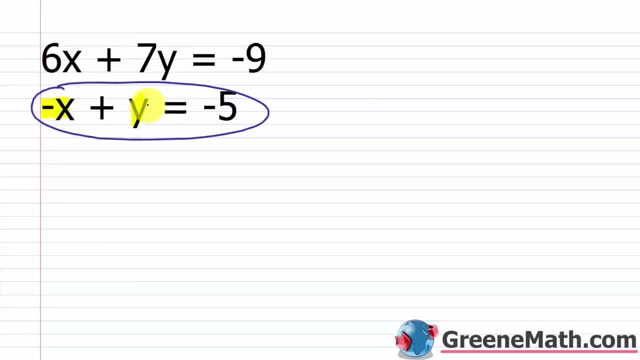 those. it's going to be quickest for me to use the y variable because the coefficient is one, So it's very easy to solve that. for y, I have negative x plus y equals negative five. just add x to both sides of the equation, So that's gone And I have y equals negative five And I have y equals negative. 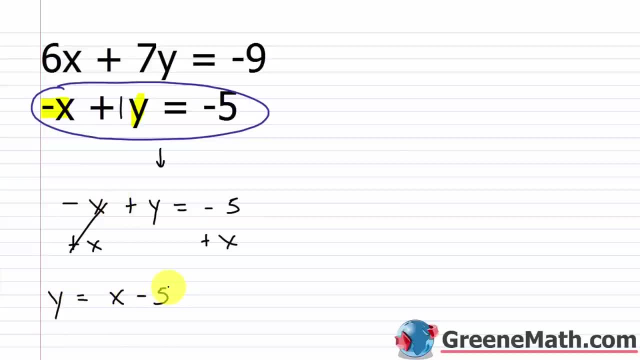 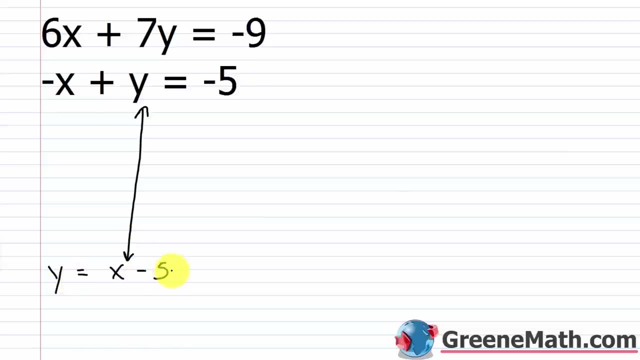 is equal to x minus 5.. So please understand at this point that these two equations are the exact same. This is the same as this. I just transformed it. It's solved for y. Now what does that mean? y equals x minus 5?. 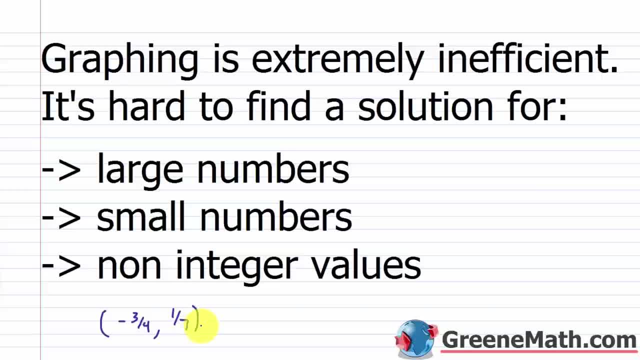 It's very hard to graph that. I know you can use a graphing calculator or a computer program, but if you're using a sheet of paper like most of you are gonna do on a test, it's not very efficient or very effective at all. 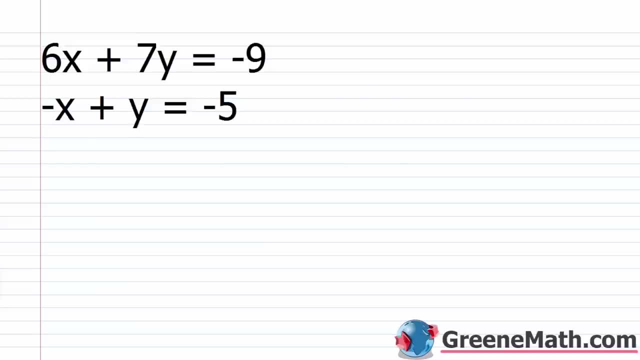 So kind of the next thing we do is turn to an algebraic method. We got the concept down. We understand about a system of linear equations and what the solution means, but we need another way to kind of attack this type of problem. So with substitution, I'm basically going to substitute in for one of the variables and create a linear equation in one variable. 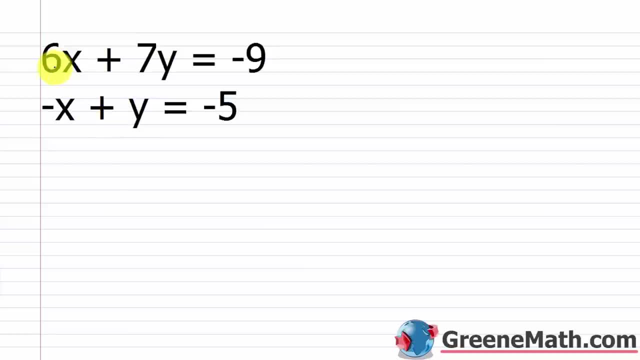 So let me kind of go deeper into that. Let's say I have this problem 6x plus 7y equals 1. So I'm gonna go ahead and do that. Let's say I have this problem 6x plus 7y equals negative 9 and negative x plus y equals negative 5. What I can do is I can solve one of the equations for one of the variables. Now, it doesn't matter which variable you pick and it doesn't matter which equation you start out with, but it's generally gonna be easier if you look for a variable that has a coefficient of one, that's the easiest, or the second easiest would be negative one. 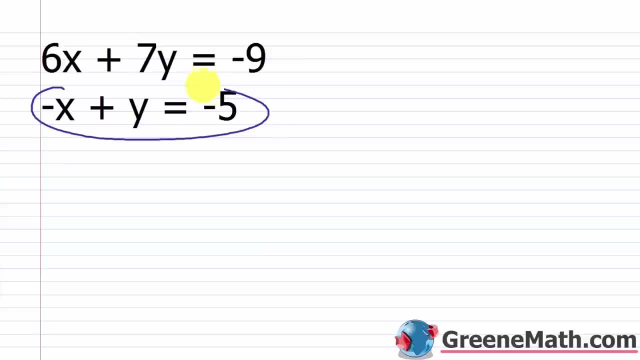 If I look at this equation here, what I see is that I have a coefficient on the y variable of one. I have a coefficient on the x variable of negative one. So I can use either of those. It's gonna be quickest for me to use the y variable because the coefficient is one. So it's very easy to solve that for y. I have negative x plus y equals negative five. Just add x to both sides of the equation. That's gone. 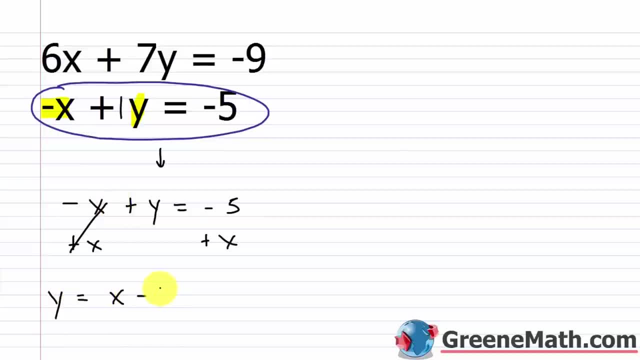 And I have y is equal to, x minus five. 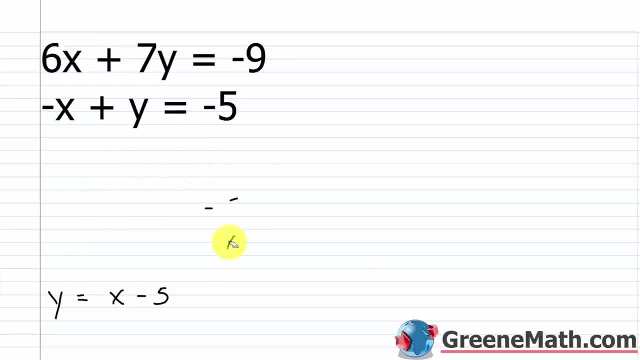 So please understand at this point that these two equations are the exact same. This is the same as this. I just transformed it. It's solved for y. 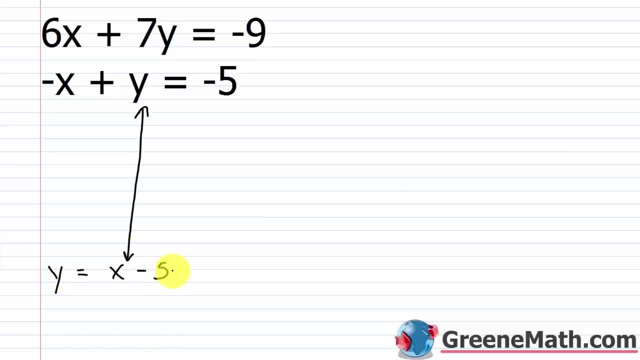 Now, what does that mean? Y equals x minus five. 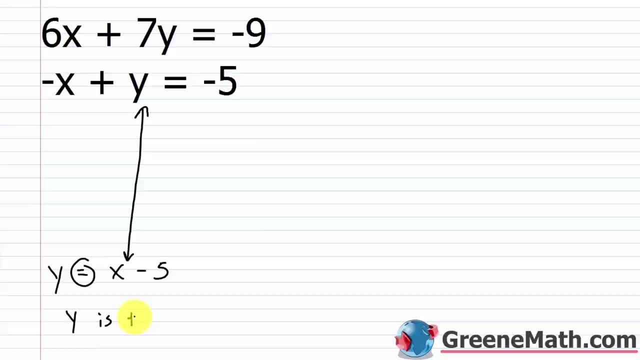 I'm saying that y, y is the same 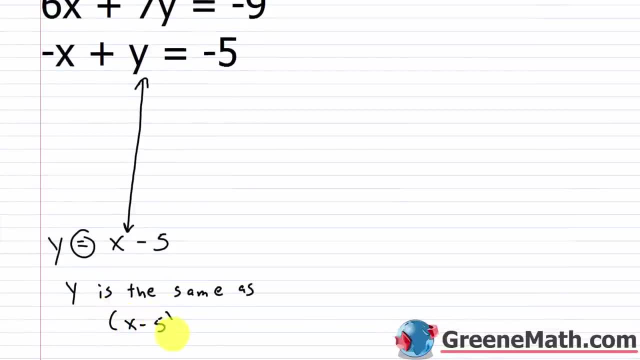 as the quantity x minus five. Those two are the same. So in terms of money, that's a good way to explain it. 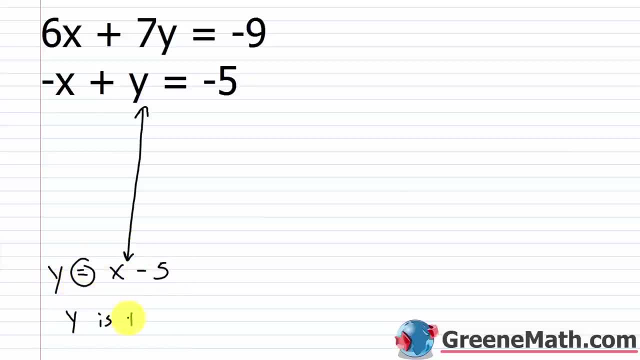 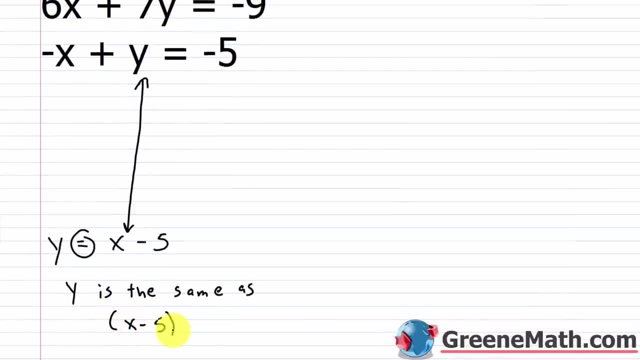 I'm saying that y is the same as the quantity x minus 5.. Those two are the same. So in terms of money, that's a good way to explain it. Let's say that I had a $100 bill And let's say that I also had five $20 bills. 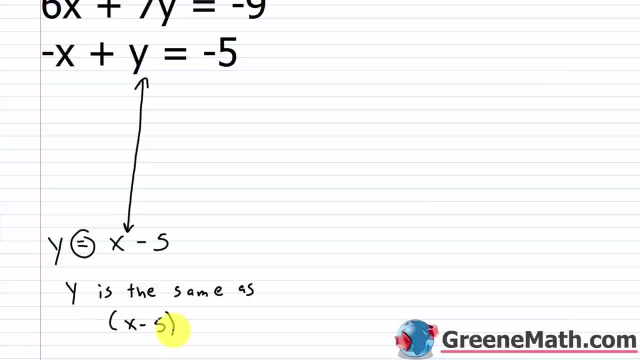 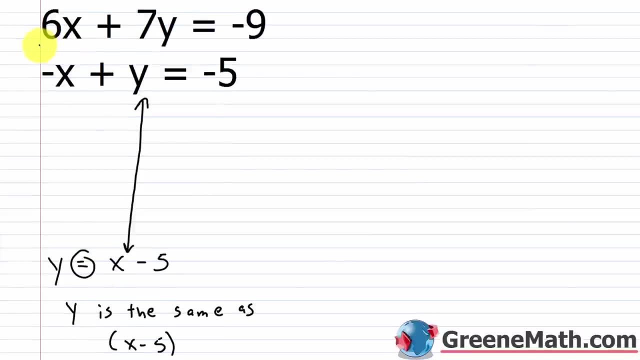 Well, they're the same in terms of value, They just look different. So these are the same, They just look different. So, because they're the same, I can go into this other equation here and I can plug in for y. 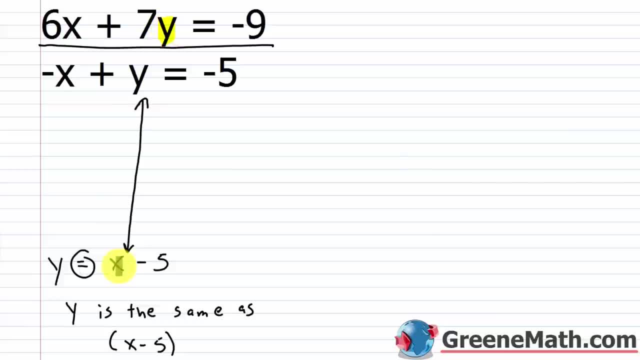 I can plug in for y. So where I see a y, I'm going to plug in an x minus 5. Because that's what y is equal to. So I'll have 6x plus 7 times. Again, I'm plugging in for y. 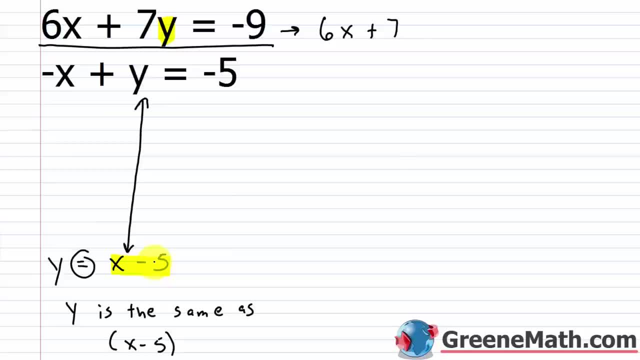 And I'm plugging in x minus 5, that quantity, So make sure you use parentheses- So the quantity x minus 5. And this equals negative 9.. So now I have a linear equation in one variable And I can solve for x and find out what that value is. 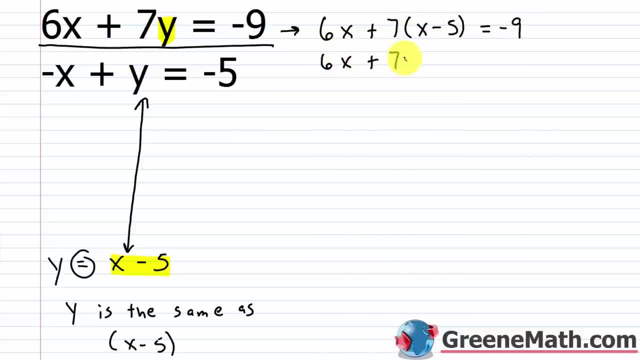 So I have: 6x plus 7 times x is 7x, And then minus 7 times 5 is 35. OK, And this is going to equal negative 9.. Combine like terms on the left: 6x plus 7x is 13x. 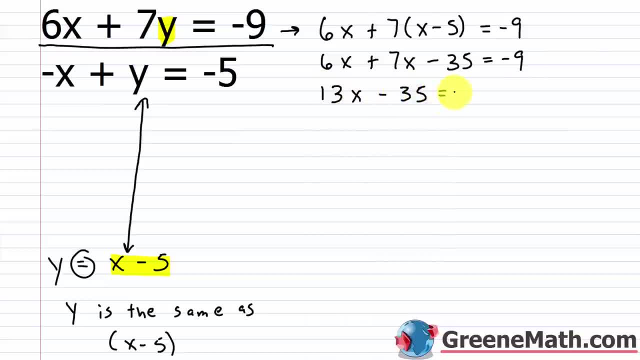 So this is: 13x minus 35 equals negative 9.. Let's add 35 to both sides of the equation, So this is going to be: 13x is equal to What's negative? 9 plus 35?? Well, that's going to be 26.. 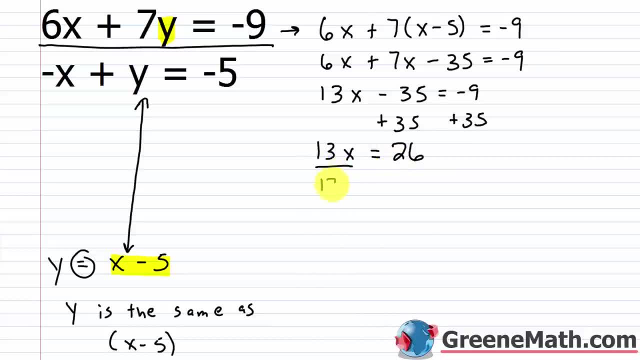 So I get 13x equals 26.. OK, That's going to be 26.. Divide both sides of the equation by 13 to get x by itself, And I get that x is equal to 2.. So at this point I have an answer. 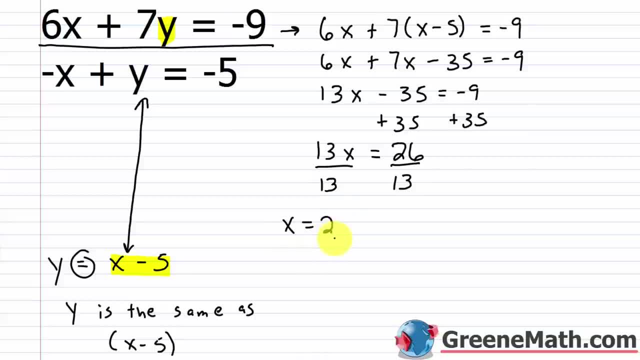 for one of the variables in the system. I know that x equals 2.. So how do I get the value for y? Well, all I need to do is plug a 2 in for x in either of the original equations. Let me erase everything. 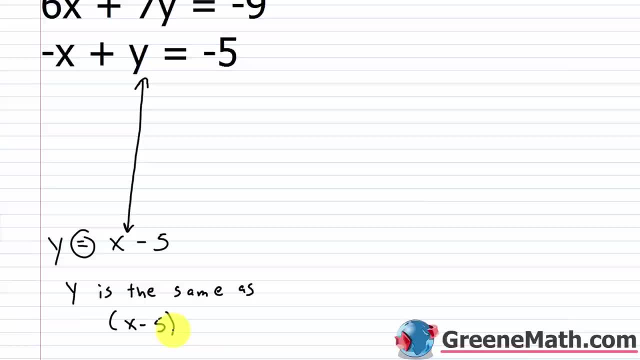 Let's say that I had a $100 bill. 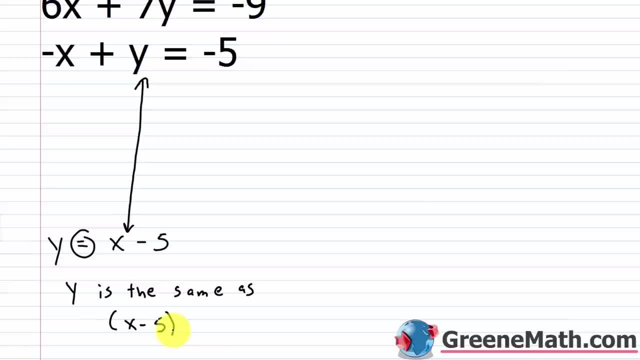 And let's say that I also had five $20 bills. Well, they're the same in terms of value. They just look different, right? So these are the same. They just look different. 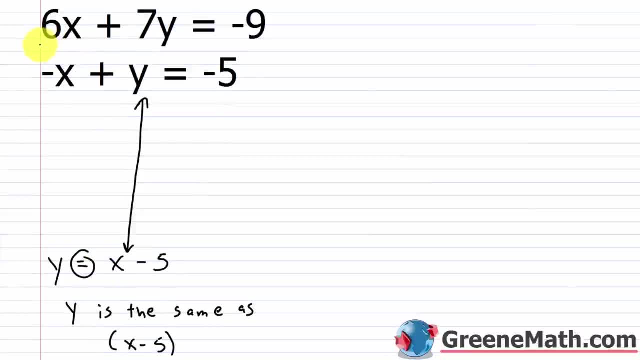 So because they're the same, I can go into this other equation here and I can plug in for y. I can plug in for y. 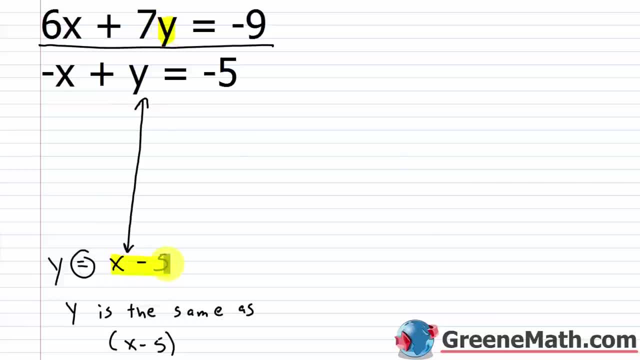 So where I see a y, I'm gonna plug in an x minus five, because that's what y is equal to. 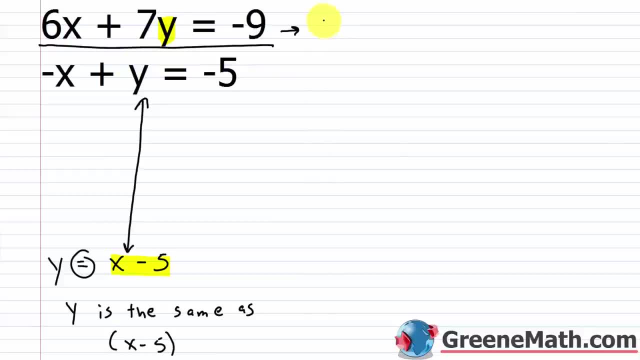 So I'll have six x plus seven times. 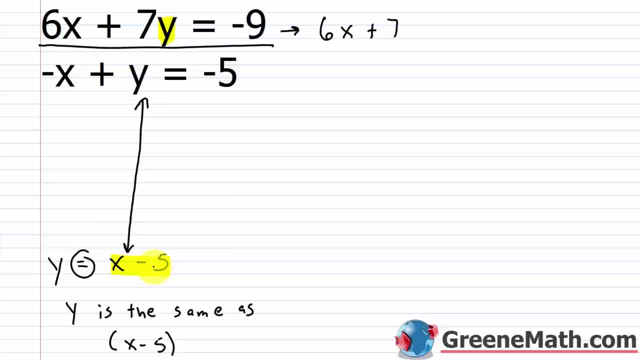 Again, I'm plugging in for y and I'm plugging in x minus five, that quantity. So make sure you use parentheses. 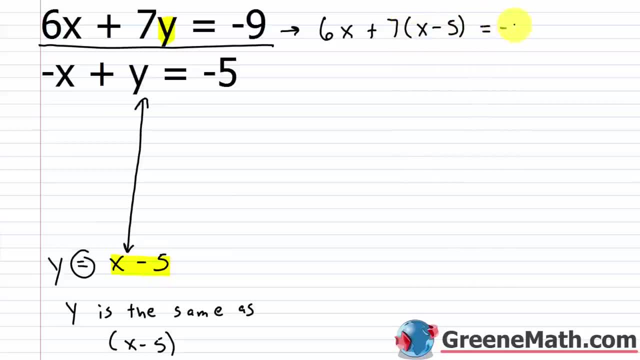 So the quantity x minus five, and this equals negative nine. 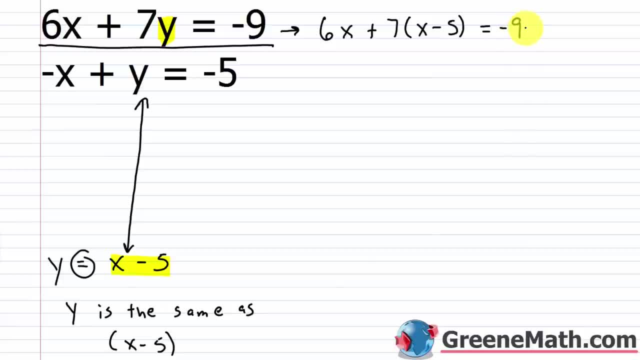 So now I have a linear equation in one variable and I can solve for x and find out what that value is. 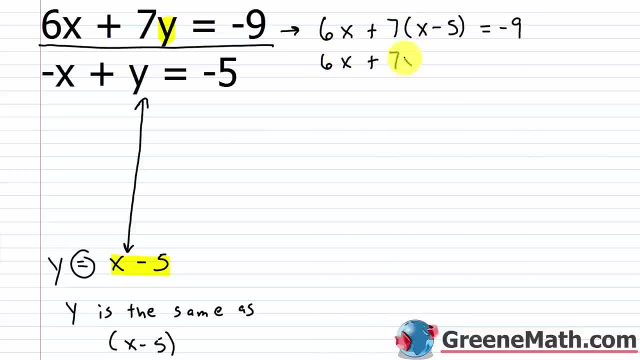 So I have six x plus seven times x is seven x, minus seven times five is 35. Okay, and this is gonna equal negative nine. Combine like terms on the left. Six x plus seven x is 13 x. So this is 13 x minus 35 equals negative nine. Let's add 35 to both sides of the equation. 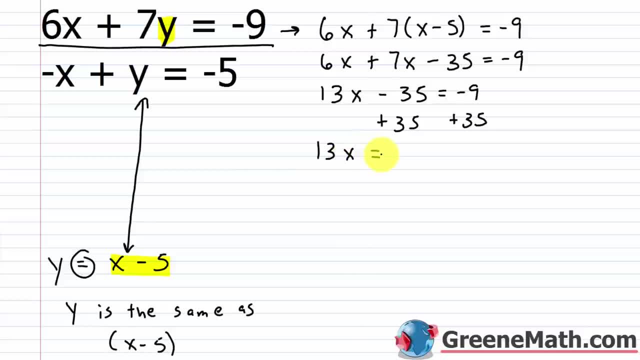 So this is gonna be 13 x is equal to, what's negative nine plus 35? 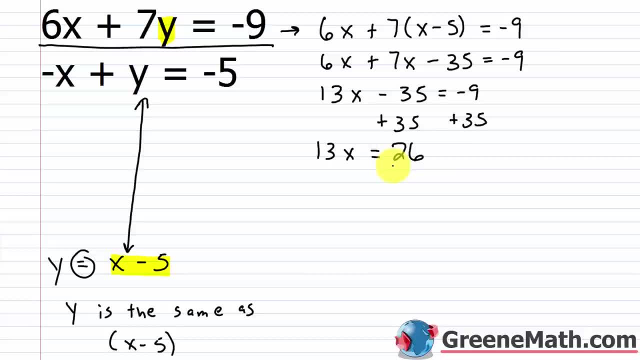 Well, that's gonna be 26. So I get 13 x equals 26. So I get 13 x equals 26. Divide both sides of the equation by 13 to get x by itself. And I get that x is equal to two. 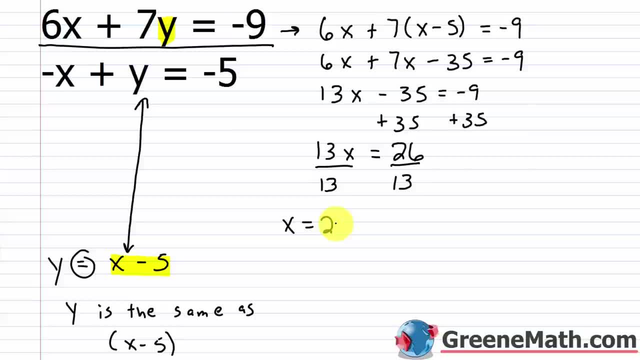 So at this point, I have an answer for one of the variables in the system. 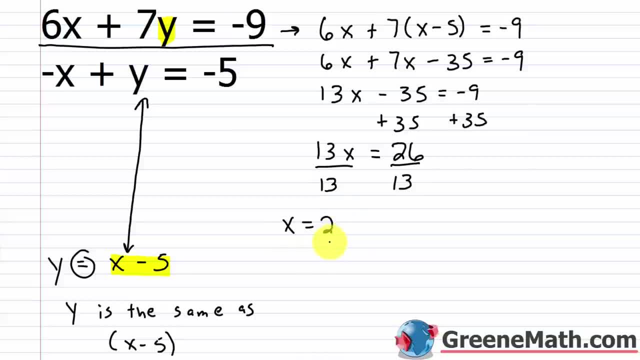 I know that x equals two. So how do I get the value for y? 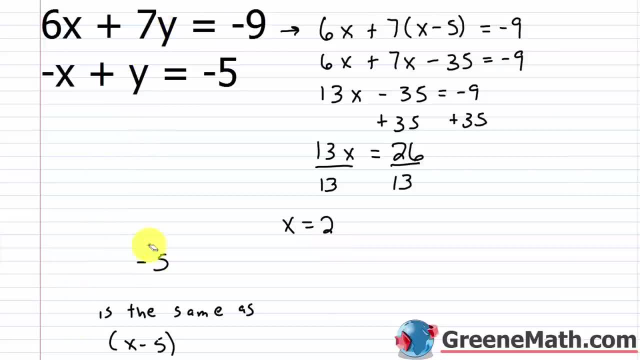 Well, all I need to do is plug a two in for x in either of the original equations. Let me erase everything. 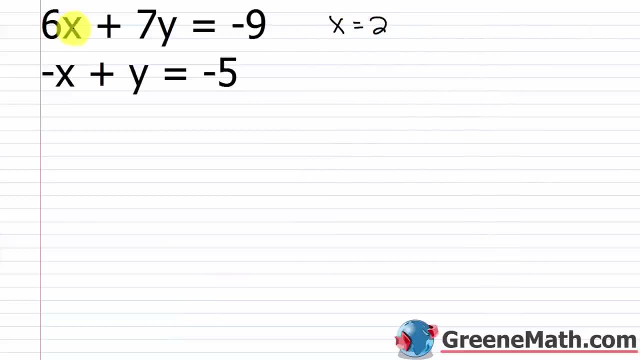 So again, I know that x equals two. So I could plug that in here or here. 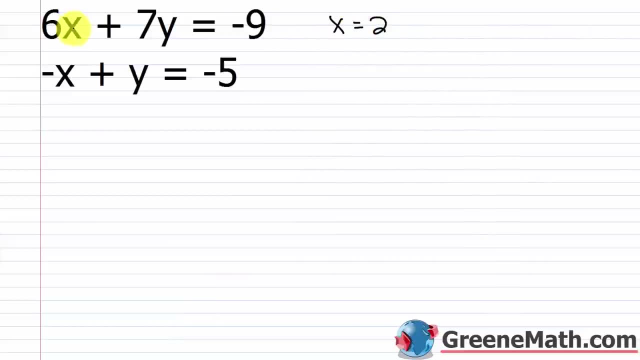 So again, I know that x equals 2. So I could plug that in here or here, Because, remember, when I look at a system, this value for x has to work as a solution in both equations. So that means I can plug it into either one. 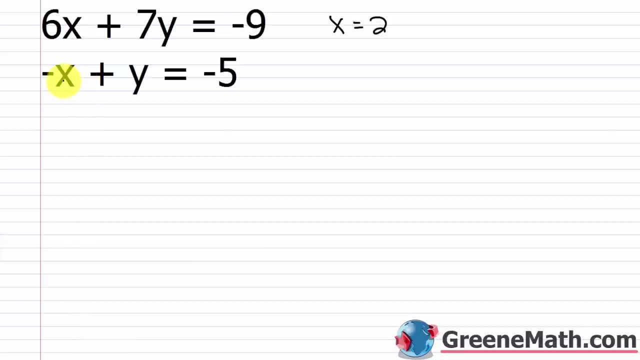 Doesn't really matter. It looks like it's going to be easier to plug it into the second one, So I'd have negative 2, right, plugging in 2 for x plus y equals negative 5.. Let's add 2 to both sides of the equation. 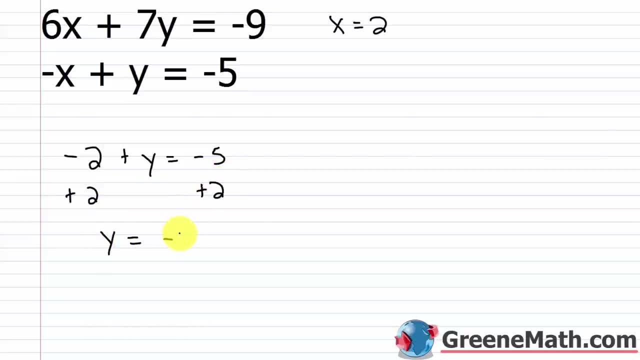 And I'm going to get: y is equal to negative. 5 plus 2 is negative 3. So x equals 2. And y is equal to negative 3. So x equals 2. And y is equal to negative 3.. 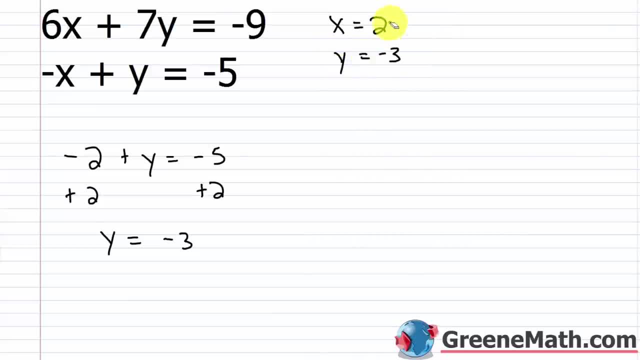 So x equals 2. And y is equal to negative 3. So x equals 2.. So x equals 2. And y is equal to negative 3.. ordered pair: this would be 2 comma negative 3. So let's erase this and put 2 comma negative 3.. 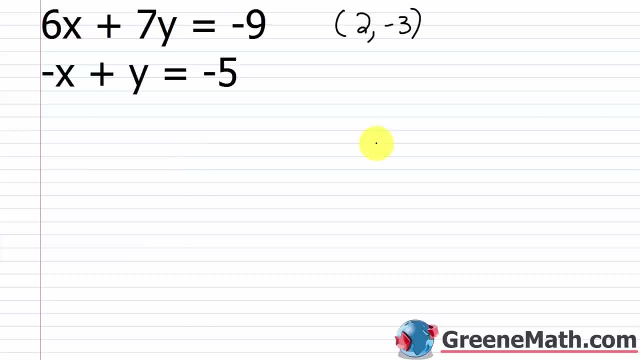 So I'm going to erase everything and we're going to check it. So remember, for this to be a solution for the system, it's got to work as a solution for both equations. It can't just work for one, it's got to work for both. So 6x, we'll put 6 times 2, plug it in a 2 for x plus 7y. 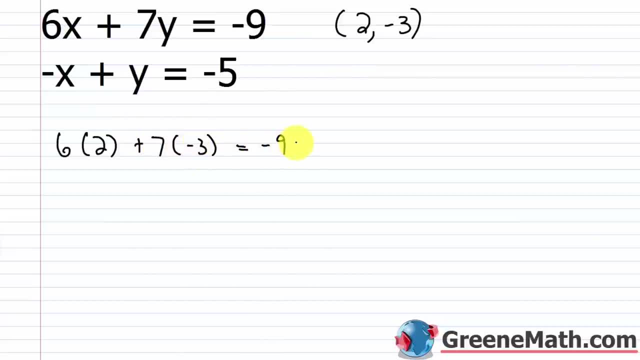 plug in a negative 3 for y equals negative 9.. 6 times 2 is 12, and then 7 times negative 3 is negative 21,. so minus 21 equals negative 9.. And that's true. 12 minus 21 is negative 9,. 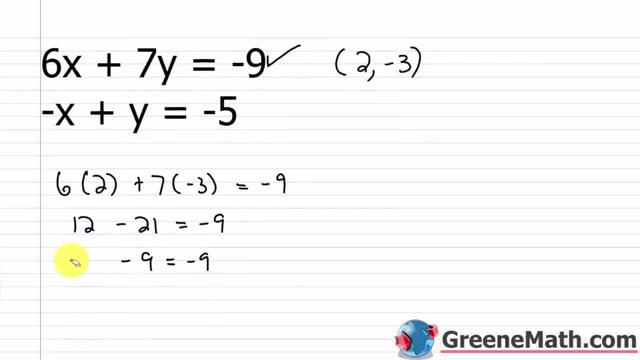 so you get negative 9 equals negative 9.. That works out All right. let's take a look at the second one. So we'd plug in a 2 for x. I have a negative out in front and then I'm going to plug. 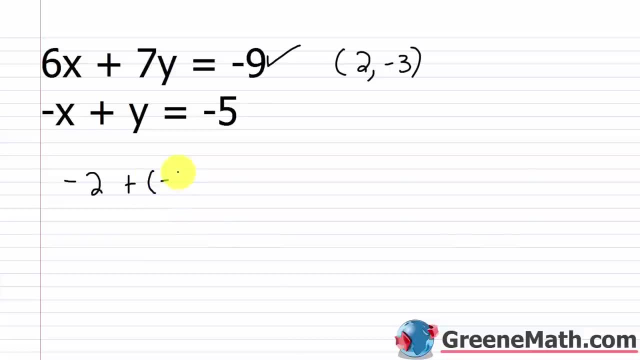 a 2 in there, plus for y I'm going to plug in a negative 3, and this should equal negative 5, and of course it does. Negative 2 plus negative 3 is negative 5, so you get negative 5 equals. 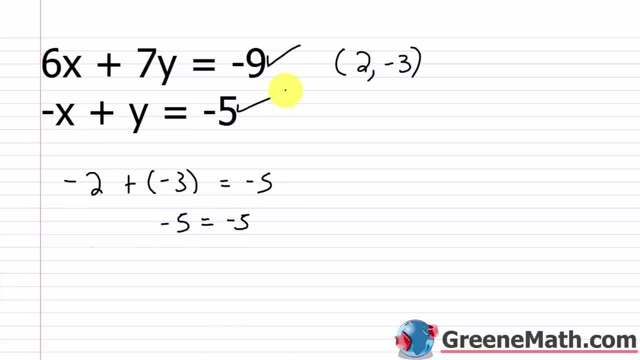 negative 5.. So again, that checks out as well. So your solution for the system here is 2 comma negative 3.. So some of you might be doubtful and you might say: well, if I had solved another one of the equations for another variable, let's say like x, I wouldn't have got the same answer. 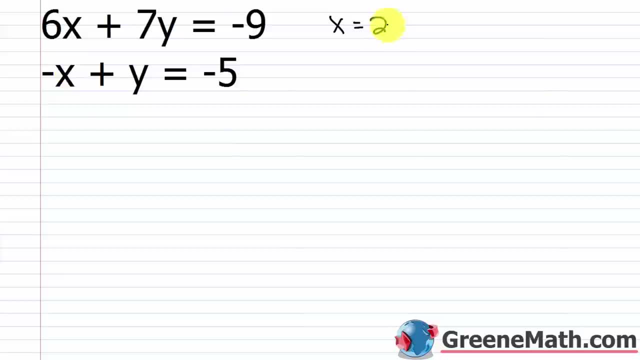 Because remember, when I look at a system, this value for x has to work as a solution in both equations. 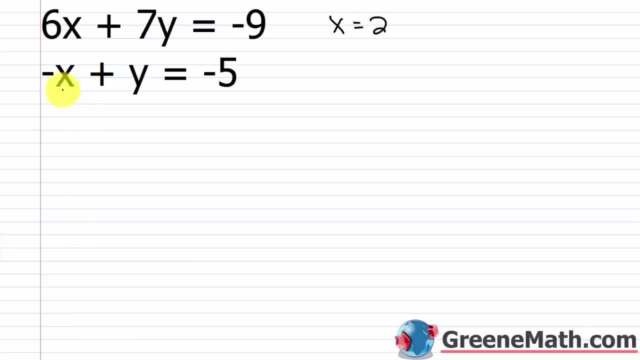 So that means I can plug it into either one. Doesn't really matter. It looks like it's gonna be easier to plug it into the second one. 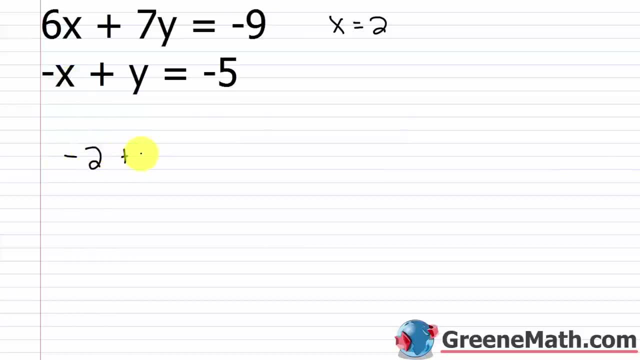 So I'd have negative two, right? Plugging in two for x plus y equals negative five. Let's add two to both sides of the equation. And I'm gonna get y is equal to negative five plus two is negative three. 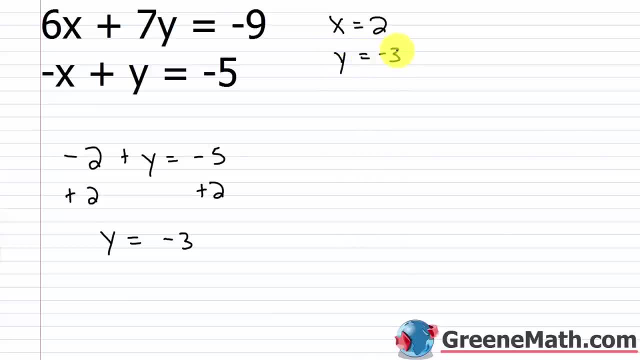 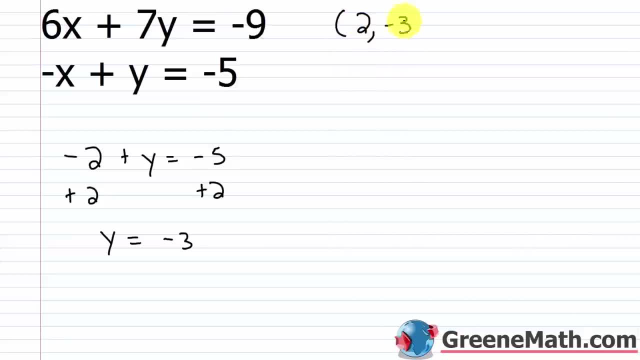 So let's erase this and put two comma, negative three. 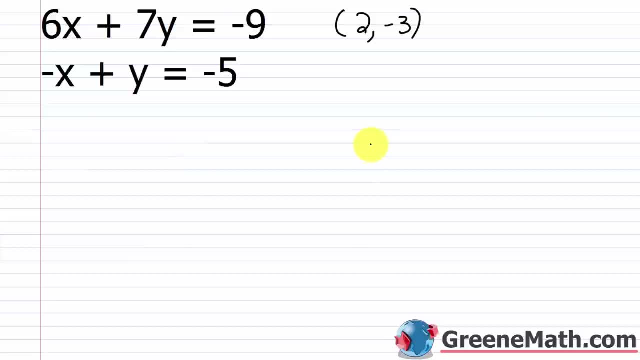 So I'm gonna erase everything and we're gonna check it. So remember, for this to be a solution for the system, it's gotta work as a solution for both equations. It can't just work for one. It's gotta work for both. 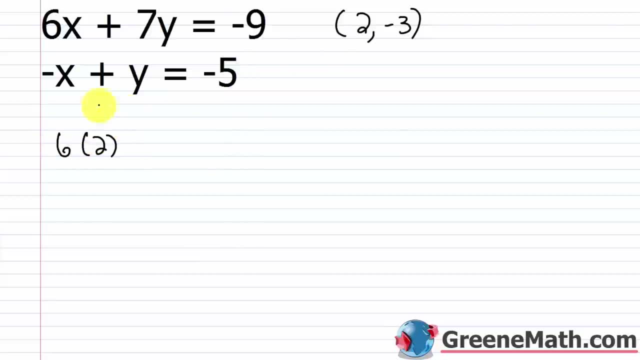 So 6x, we'll put six times two. Plug it in at two for x. Plus seven y. Plug it in at negative three for y, equals negative nine. 6 times 2 is 12, and then 7 times negative 3 is negative 21, so minus 21 equals negative 9, 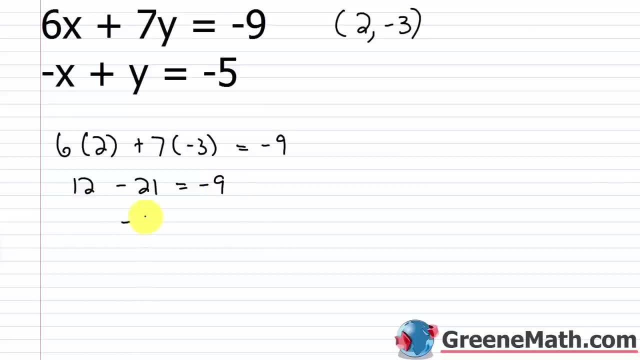 and that's true. 12 minus 21 is negative 9, so you get negative 9 equals negative 9. That works out. 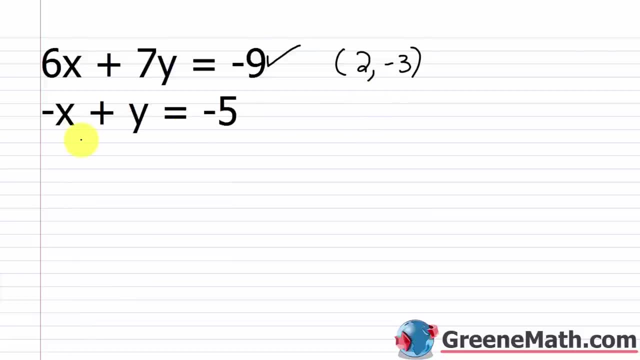 All right, let's take a look at the second one. So we'd plug in a 2 for x. I have a negative out in front, and then I'm going to plug a 2 in there, plus for y, I'm going to plug in a negative 3, and this should equal negative 5, and of course it does. Negative 2 plus negative 3 is negative 5, 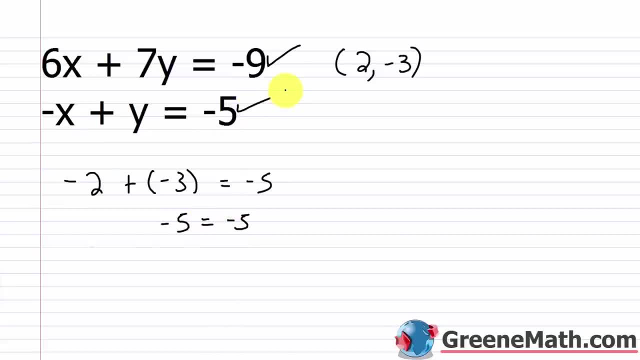 so you get negative 5 equals negative 5, so again that checks out as well. So your solution for the 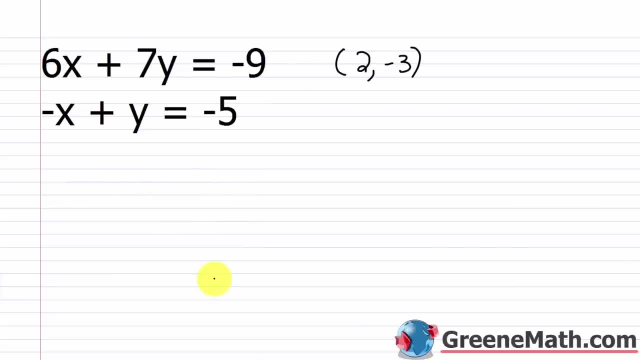 system here is 2 comma negative 3. So some of you might be doubtful, and you might say, well, if I had solved another one of the equations for another variable, let's say like x, I wouldn't have got the same answer. Well, you would have. The reason that I solved this equation for y is 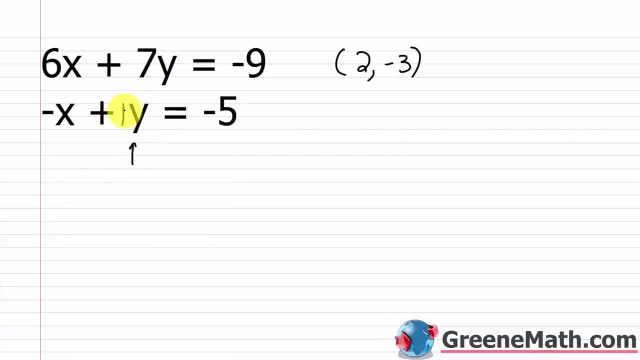 because y had a coefficient of 1. When you look at your section in your book on substitution, they're going to 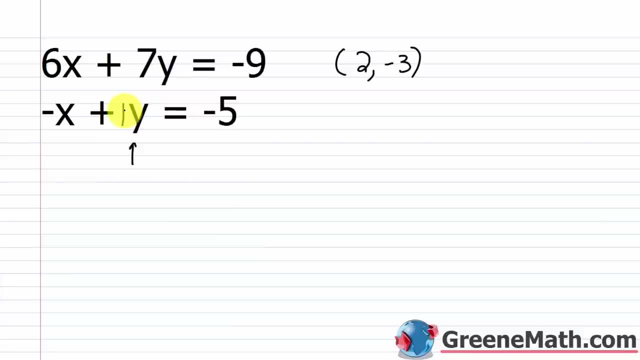 teach you to look for variables that have a coefficient of 1 or negative 1, because they're really easy to solve an equation for that. But I'm going to go ahead and solve this first equation 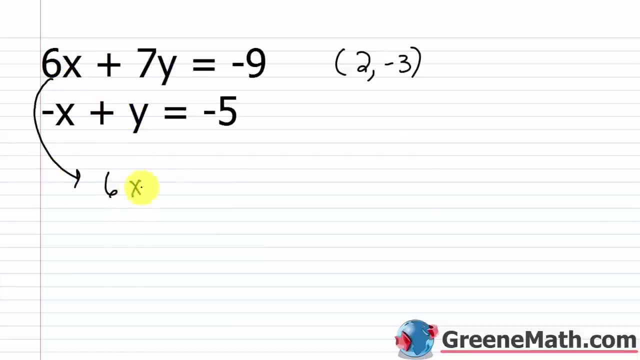 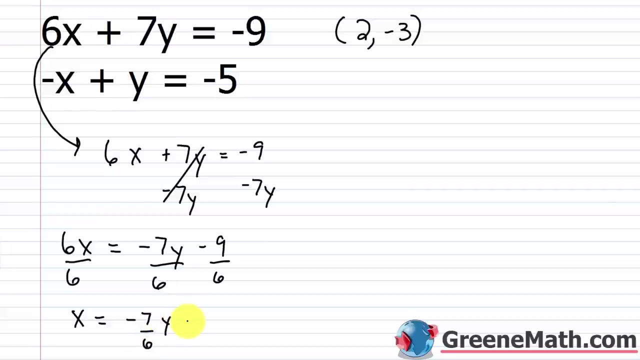 for x and restart the problem. So 6x plus 7y equals negative 9. I would subtract 7y away from each side. That would go away. I'd have 6x is equal to negative 7y minus 9. Divide both sides by 6. Again, the coefficient of x. And so I'd have x is equal to negative 7y minus 9. And so I'd have x is equal to negative 7, 6y minus, for 9 over 6, they're both divisible by 3. So this would 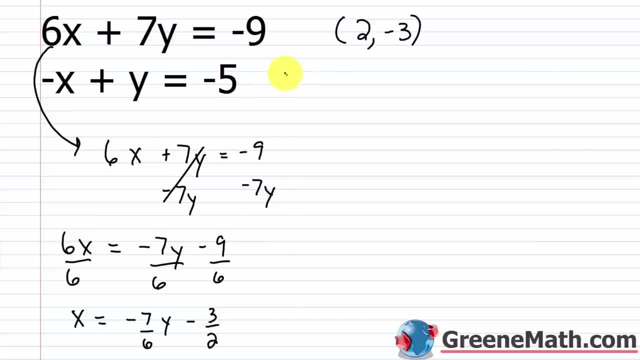 be 3 halves. All right. So x equals negative 7, 6y minus 3 halves. So once I know what x is equal to, I can plug in for x in the other equation. So I started with this one. I'm going to plug into this one. So instead of an x there, I'm going to have a negative. 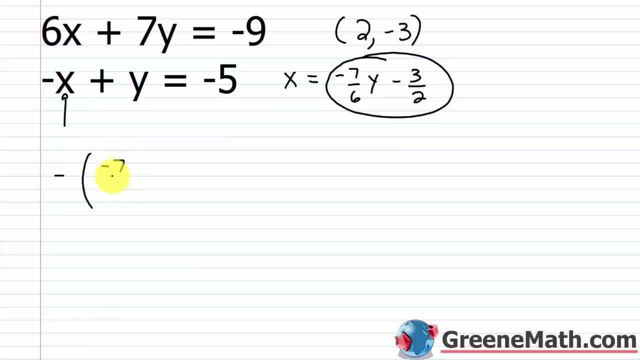 And then I'm going to have negative 7, 6y minus 3 halves. Then plus y equals negative 5. So I have a linear equation of one variable, and that variable is y. So a negative out in front, you can think of that as a negative 1 out in front. Just change the sign of each term inside the parentheses. So instead of negative 7, 6, I'd have 7, 6. Then y. Instead of minus 3 halves, I'd have plus 3 halves. 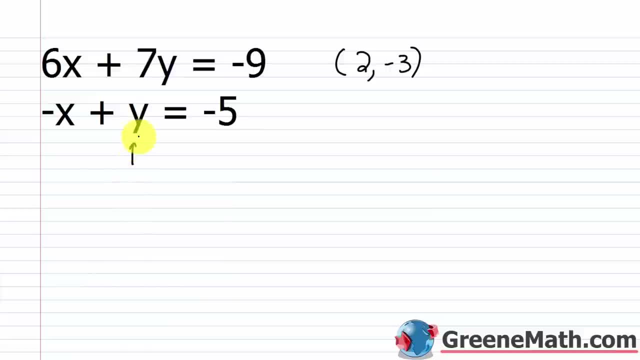 Well, you would have. The reason that I solved this equation for y is because y had a coefficient of 1.. When you look at your section in your book on substitution, they're going to teach you to look for variables that have a coefficient of 1 or negative 1, because they're really easy to solve. 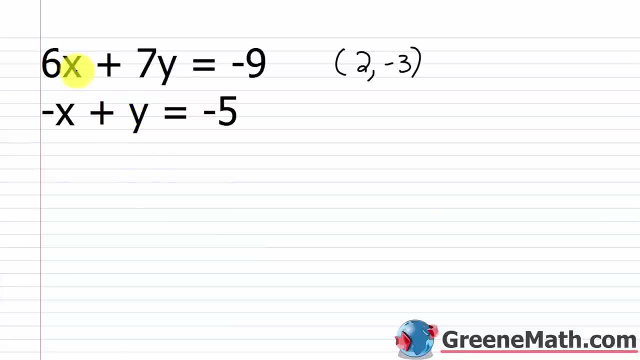 an equation for that, But I'm going to go ahead and solve this first equation for x and restart the problem. So 6x plus 7y equals negative 9.. I would subtract 7y away from each side. That would go away. I'd have: 6x is equal to negative 7y minus 9.. 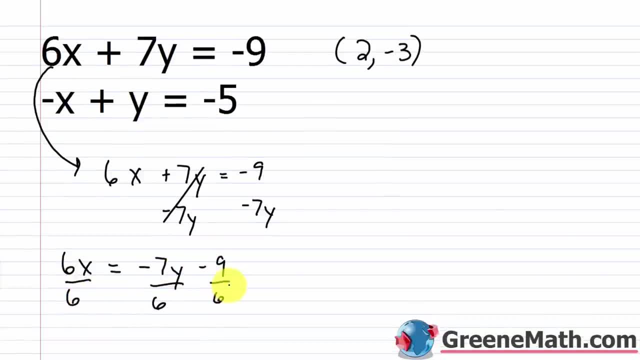 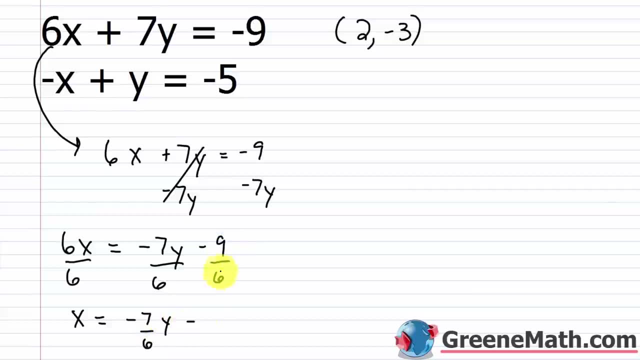 Divide both sides by 6.. Again the coefficient of x- And so I'd have x- is equal to negative 7, 6y minus for 9 over 6, they're both divisible by 3.. So this would be 3 halves. All right, So x equals. 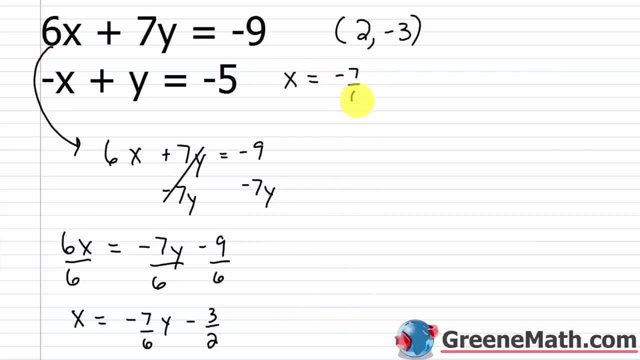 x equals negative 7, 6y minus 3 halves. So once I know what x is equal to, I can plug in for x in the other equation. With this one, I'm going to plug into this one. So instead of an x there, I'm going to have a. 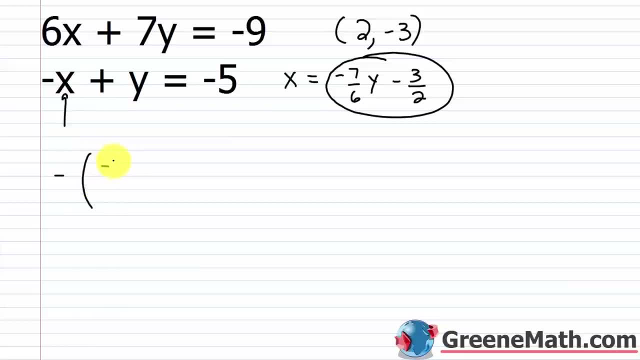 negative. And then I'm going to have negative 7, 6y minus 3 halves. then plus y equals negative 5.. So I have a linear equation of one variable, and that variable is y, So a negative out in front. 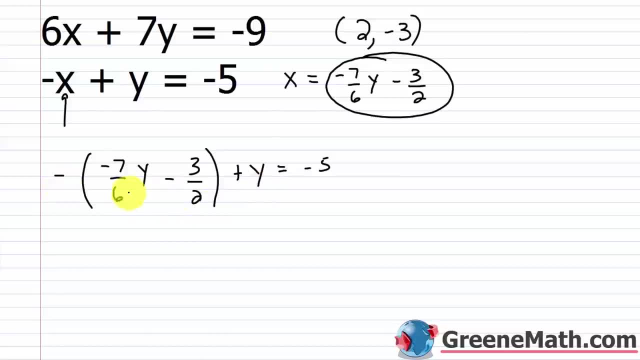 you can think of that as a negative 1 out in front. Just change the sign of each term inside the parentheses. So instead of negative 7- 6, I'd have 7- 6.. And then y. instead of minus 3 halves I'd have plus 3 halves, And then plus y equals negative 5.. 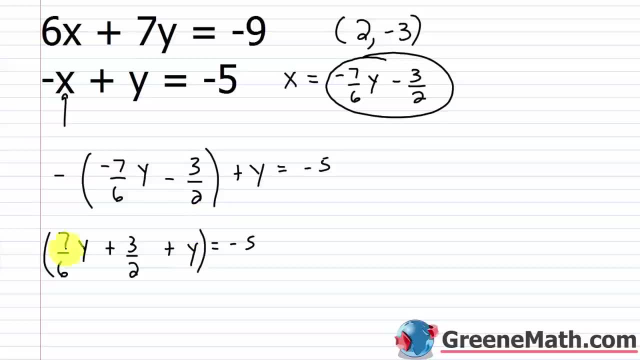 If I want, I could multiply both sides of the equation by 6 to clear the denominators. So 6 times 7, 6y would be 7y. plus 6 times 3 halves The 6 would cancel with the 2 and give me a 3.. 3 times 3 is 9.. Plus 6 times y is 6y And this equals negative 5 times. 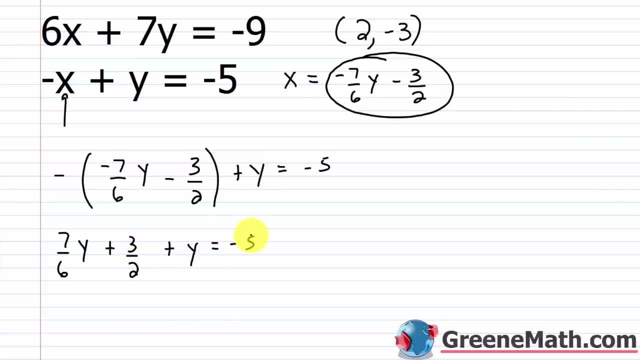 And then plus y equals negative 5. If I want, I can multiply both sides of the equation by 6 to clear the denominators. So 6 times 7, 6y would be 7y plus 6 times 3 halves. The 6 would cancel with the 2 and give me a 3. 3 times 3 is 9. Plus 6 times y is 6y. And this equals negative 5 times 6. That's negative 30. All right. So 7y plus 6y is 13. 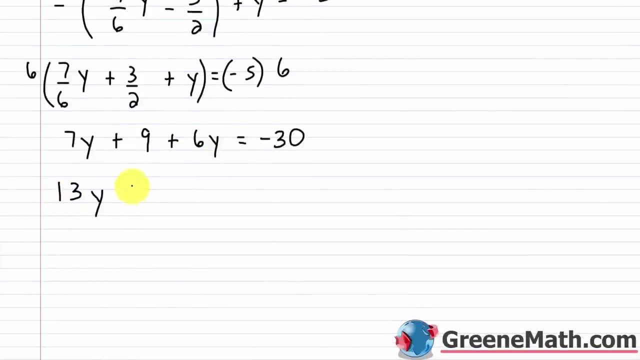 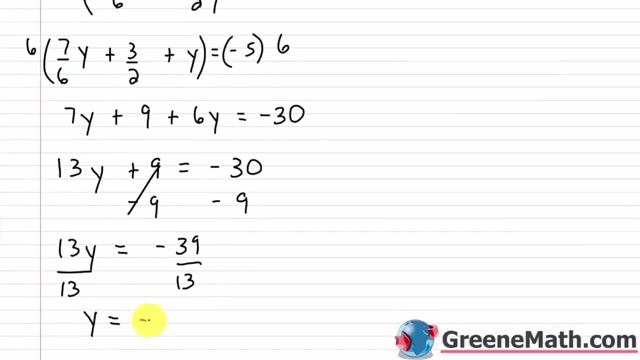 So I'll have 13y here. Then plus 9 equals negative 30. I would subtract 9 away from each side. So that's going to cancel. And I'd have 13y is equal to negative 39. As a final step, I'll divide both sides of the equation by 13. And I'm going to get that y is equal to negative 3. 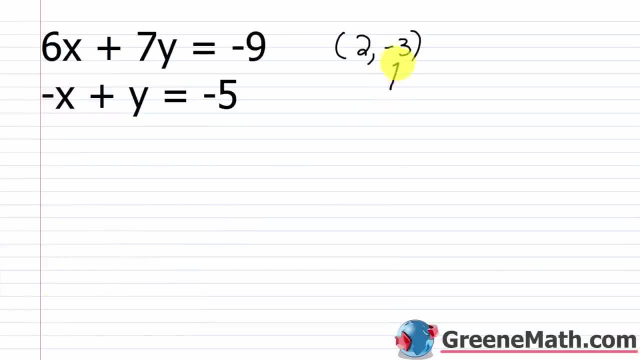 Let me erase everything. So when we come back up here, we see that we originally found that, y was negative 3. A little bit less work because we had an easier equation to kind of work with at first. But we found the same answer either way. And then again, you have negative 3. So you go ahead and plug it into either of the original equations. And you will get 2 as a result for x. 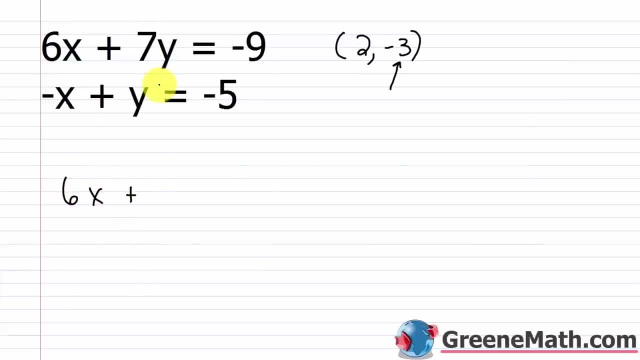 So let's do that real quick. So 6x plus 7 times negative 3 is negative 21. So plus negative 21 equals negative 9. And we'd add 21 to both sides of the equation. 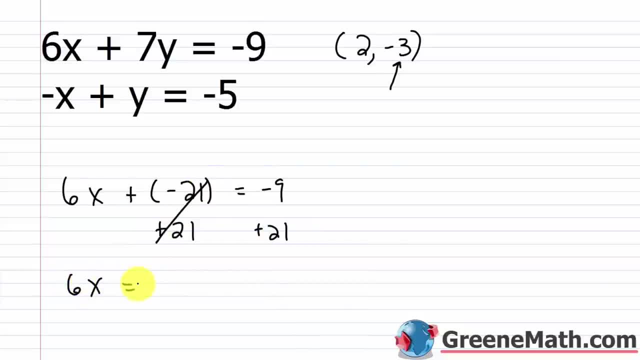 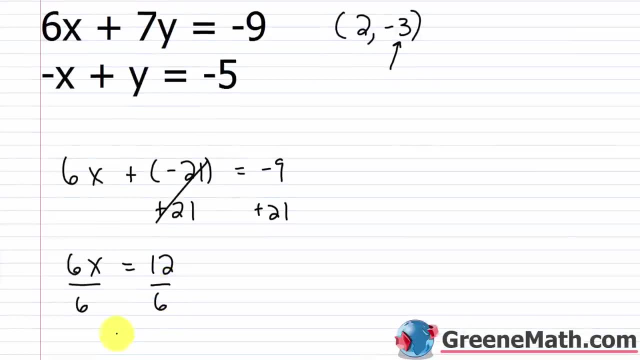 So this would cancel. You'd have 6x is equal to negative 9 plus 21 is going to give me 12. Divide both sides of the equation by 6. And of course, you get x equals 2, which is exactly what you had right there. 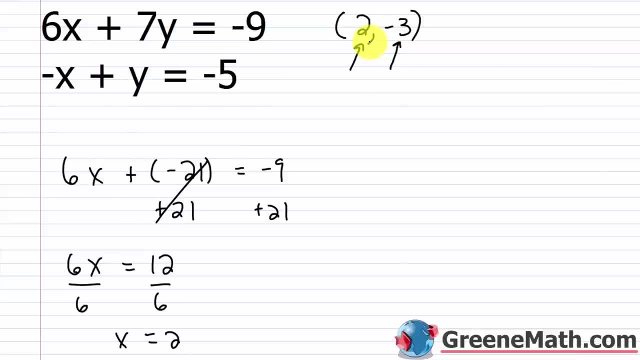 So either way you do it, you get the same answer. The solution for your system is 2 comma negative 3. Now, I want to eliminate one source of confusion before we move on to look at another problem. Once we find the value for one of the variables, I told you clearly that you can plug it in for either equation, either original equation, and get the result for the other unknowns. So in other words, if I figured out that y was negative 3, I could plug that in here or here, doesn't matter, and solve for the unknown x. And that 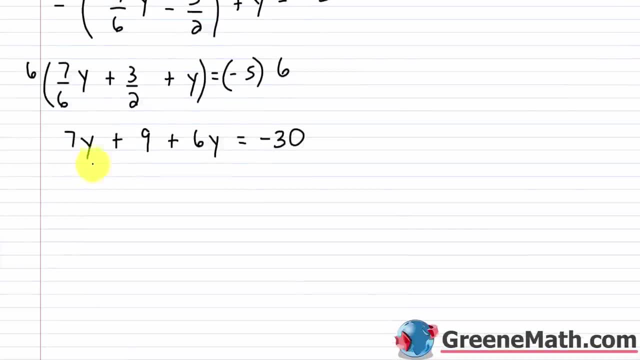 6. That's negative 30. All right, So 7y plus 6y is 13y, So I'll have 13y here. Then plus 9 equals negative 30. I would subtract 9 away from each side, So that's going to cancel And I'd have 13y. 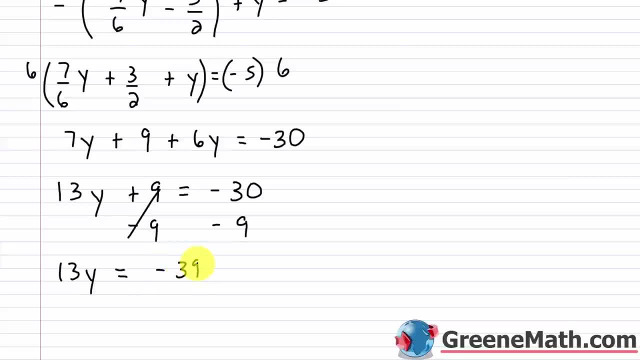 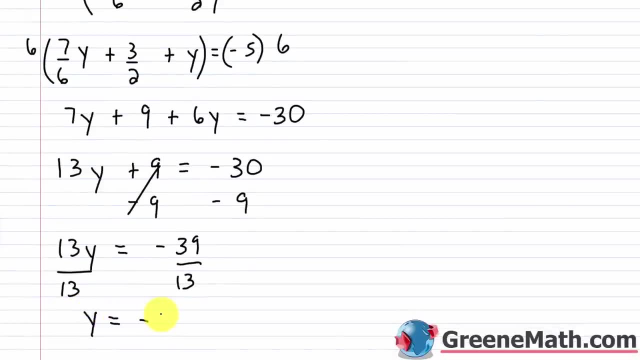 is equal to negative 39.. As a final step, I'll divide both sides of the equation by 13.. And I'm going to get that y is equal to negative 30.. Let me erase everything. So when we come back up here, we see that we originally found that y was. 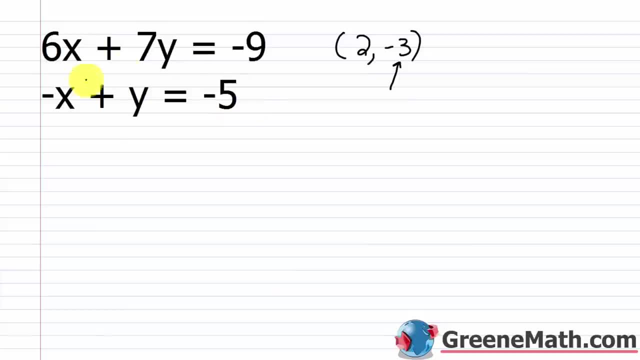 negative 3.. A little bit less work because we had an easier equation to kind of work with at first, But we found the same answer either way And then again you have negative 3.. So you go ahead and plug it into either of the original equations And you will get 2 as a result for x. So let's 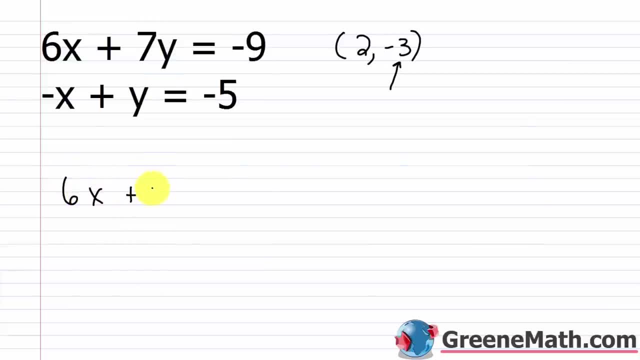 do that real quick. So 6x plus 7 times negative 3 is negative 21.. So plus negative 21 equals negative 9. And we'd add 21 to both sides of the equation, So this would cancel. You'd have 6x is equal to. 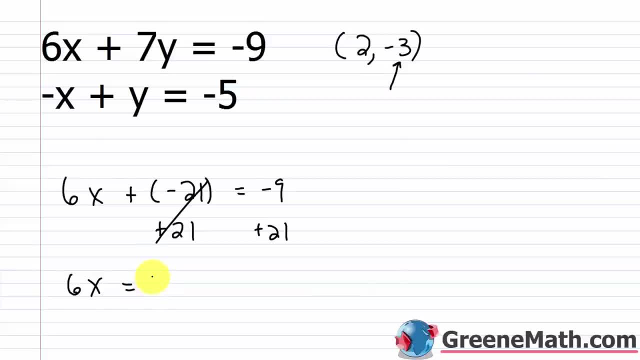 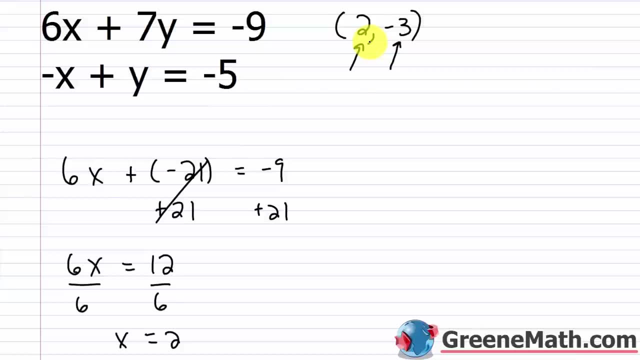 negative 9 plus 21 is going to give me 12.. Divide both sides of the equation by 6. And, of course, you get x equals 2, which is exactly what you had right there. So either way you do it. 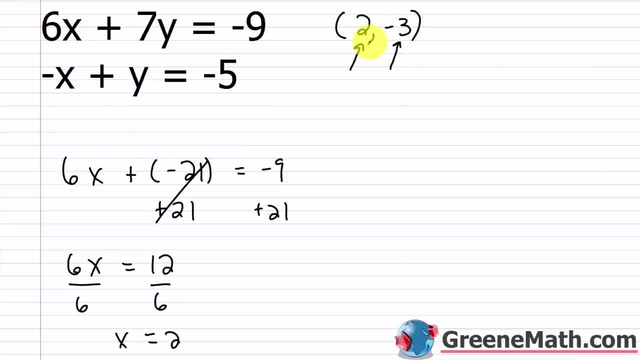 you get the same answer. The solution for your system is 2 comma negative 3.. Now I want to eliminate one source of confusion before we move on to look at another problem. Once we find the value for one of the variables, I told you clearly that you can plug it in. 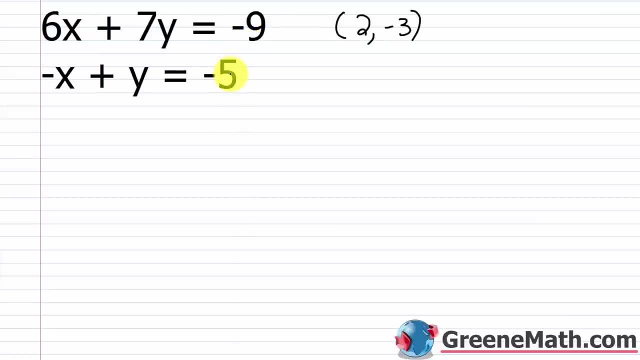 for either equation right, either original equation, and get the result for the other unknown. So in other words, if I figured out that y was negative 3, I could plug that in here or here doesn't matter- and solve for the unknown x, And that would be the x. that's the. 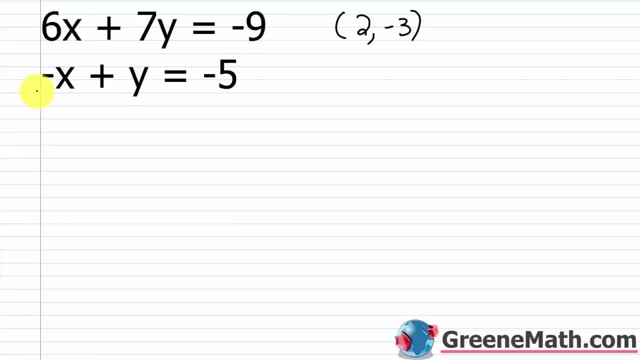 solution to the system. One thing that's a little different: if, when I originally take an equation and I solve it for one of the variables, I can't plug it back into that one right? So if you do that, you're going to get 0 equals 0. And let me show you that real fast before we move on. 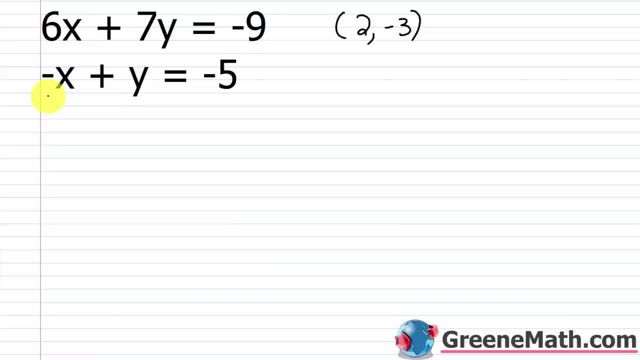 would be the x that's the solution to the system. One thing that's a little different, if when I originally take an equation and I solve it for one of the variables, I can't plug it back into that one. 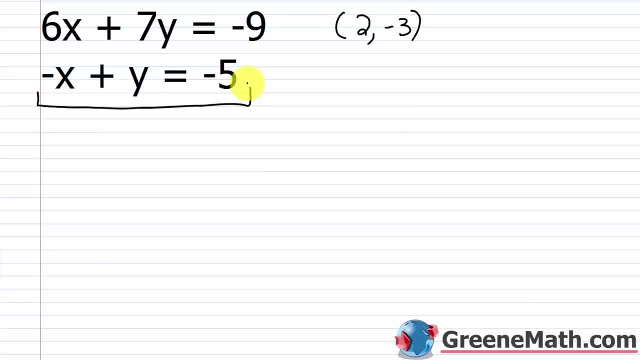 right so if you do that you're gonna get zero equals zero and let me show you that real fast before we move on because I think it's important so let's say I solve this for Y so Y equals again I'd add X to both sides of the equation so X minus 5 if I plug in X minus 5 for Y there I'm just gonna get 0 equals 0 so in the first step you always want to plug into the other equation it's once you've figured out what one of the values is gonna be then you can plug it into either equation okay so I want to make sure that you understand that so let's just plug that in real quick so you can see that so you'd have negative X plus Y is equal to X minus 5 so I'm gonna plug in an X minus 5 and then equals negative 5 so negative X plus X is 0 then I have minus 5 equals negative 5 I could add 5 to both sides of the equation now we cancel and that would cancel now we get 0 equals 0 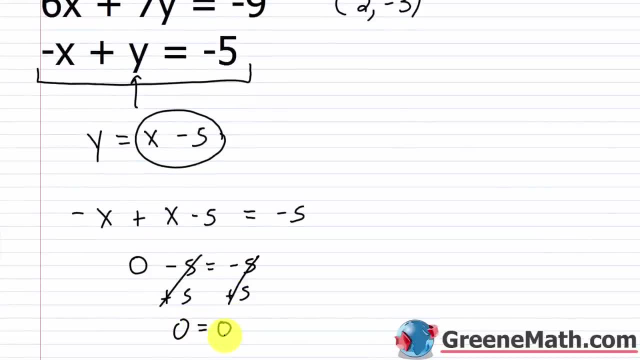 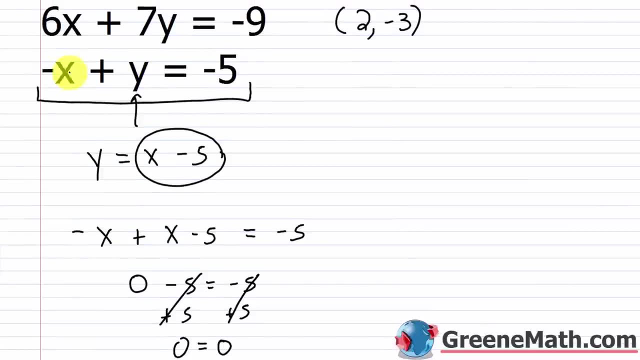 so if you end up with something like that and you're like what happened well you plug back into the equation that you just started off with and you can't do that so if you originally solve this one for Y or solve it for X you've got to 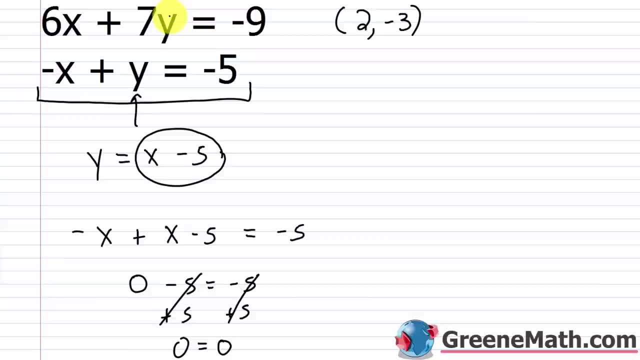 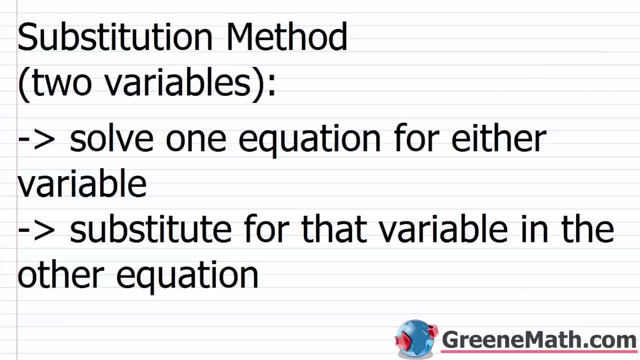 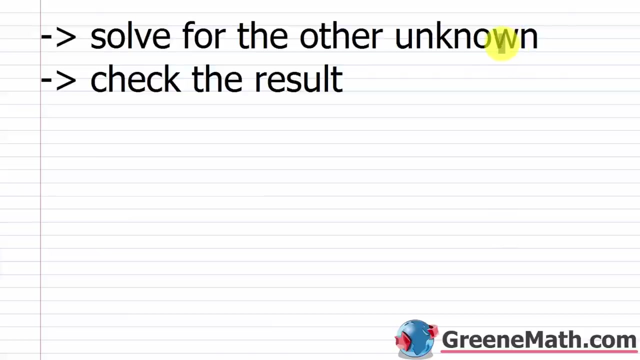 plug into the other equation to get started once you've gotten a solution for one of the variables that's when you can plug it into either one so let's look at the official procedure real quick and then we're just gonna attack a bunch of problems so substitution method with two variables so solve one equation for either variable doesn't matter which one again look for a variable with a coefficient of 1 or negative 1 then you want to substitute for that variable in the other equation again very important in the other the other equation then we're gonna solve for the other unknown right so how do we do that well once we substitute it in we get a value for one of the variables and then we can plug it back into either of the original equations and that's how we're gonna solve for the other unknown and then we just check our result remember the 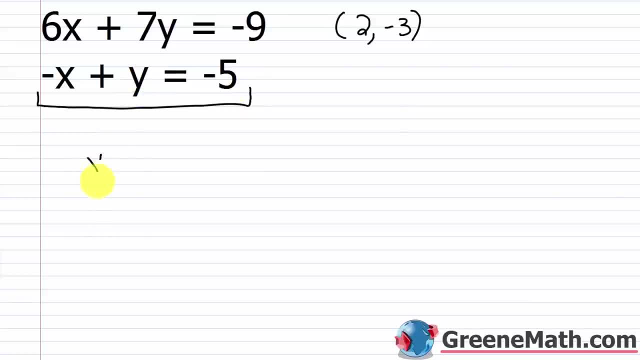 because I think it's important. So let's say I solve this for y, So y equals. again I'd add x to both sides of the equation, So x minus 5.. If I plug in x minus 5 for y, there I'm just going. 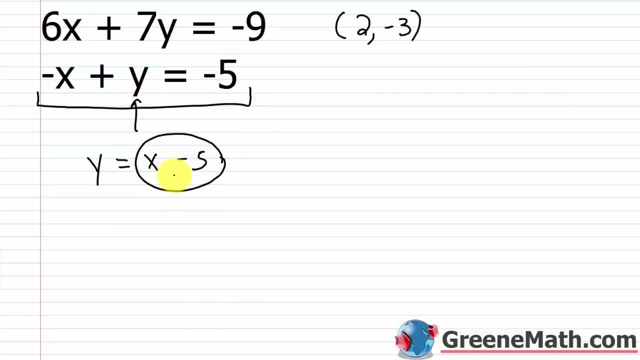 to get 0 equals 0. So in the first step you always want to plug into the other equation. It's once you've figured out what one of the values is going to be, then you can plug it into either equation. So I want to make sure that you understand that. So let's just plug that in real. 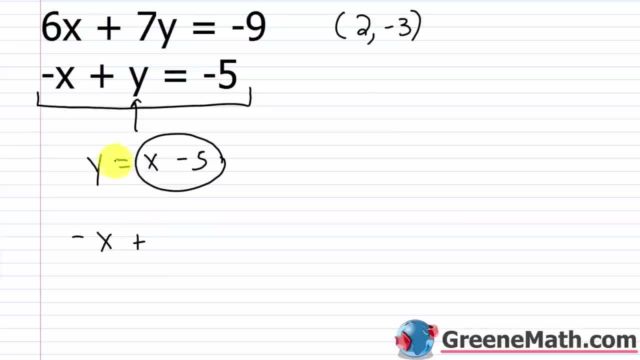 quick so you can see that. So you'd have: negative x plus y is equal to x minus 5.. So I'm going to plug in an x minus 5, and then equals negative 5.. So negative x plus x is 0. Then I have minus 5. 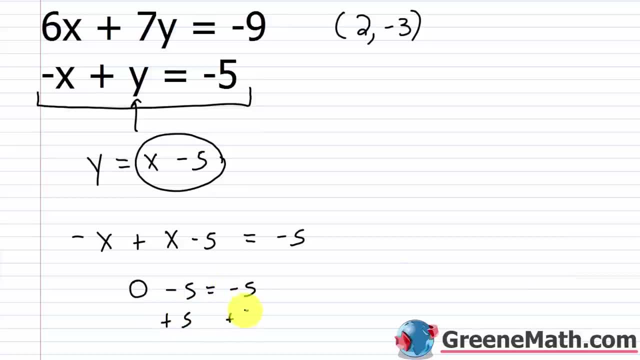 equals negative 5.. I could add 5 to both sides of the equation. That would cancel, and that would cancel And I would get 0 equals 0. So I'm going to plug in x minus 5.. So I'm going to plug in x. 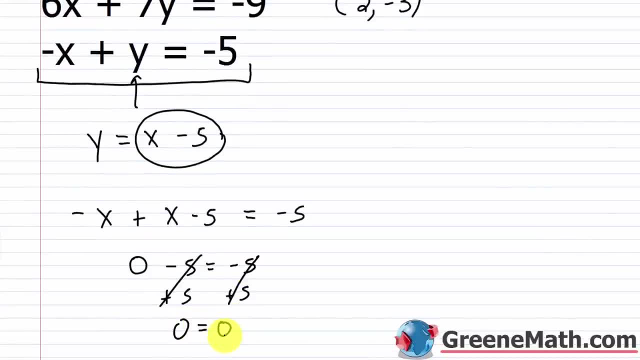 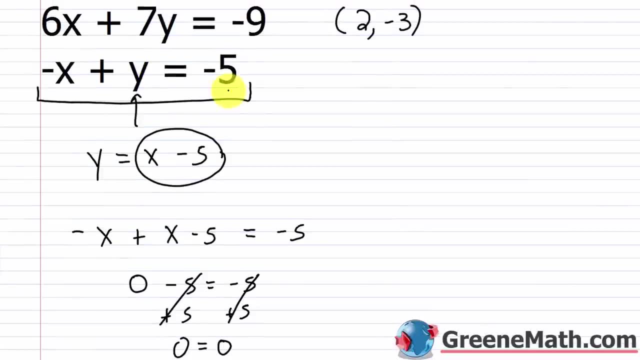 equals 0.. So if you end up with something like that and you're like what happened, Well, you plug back into the equation that you just started off with, and you can't do that. So if you originally solved this one for y, or solve it for x, you've got to plug into the other equation. 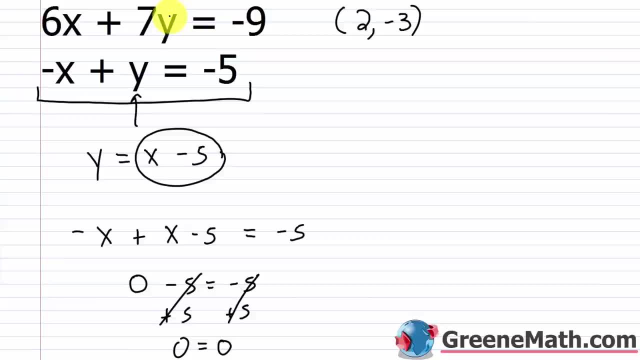 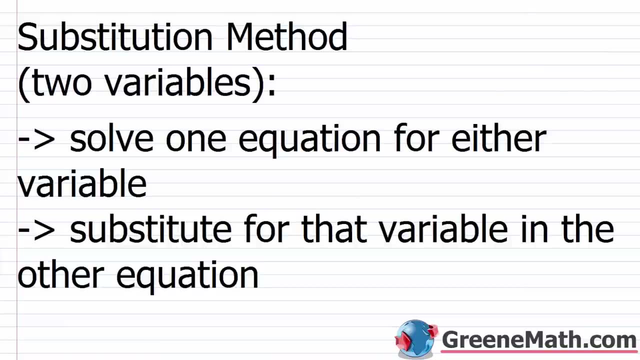 to get started Once you've gotten a solution for one of the variables, that's when you can plug it into either one. So let's look at the official procedure real quick and then we're just going to attack a bunch of problems. So, substitution method with two variables. So solve one. 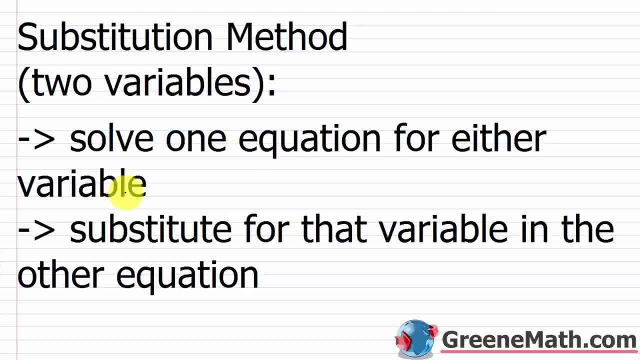 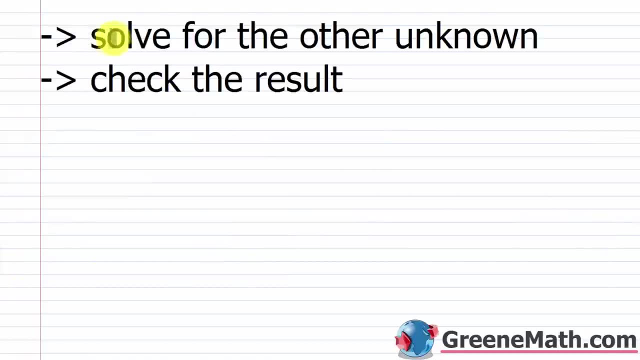 equation for either variable, It doesn't matter which one. Again, look for a variable with a coefficient of 1 or negative 1.. Then you want to substitute for that variable in the other equation- Again very important- In the other equation. Then we're going to solve for the other, unknown. 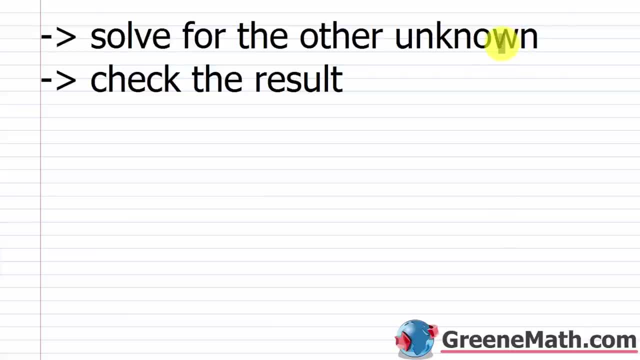 So how do we do that? Well, once we substitute it in, we get a value for one of the variables, and then we can plug it back into either of the original equations, and that's how we're going to solve for the other unknown. 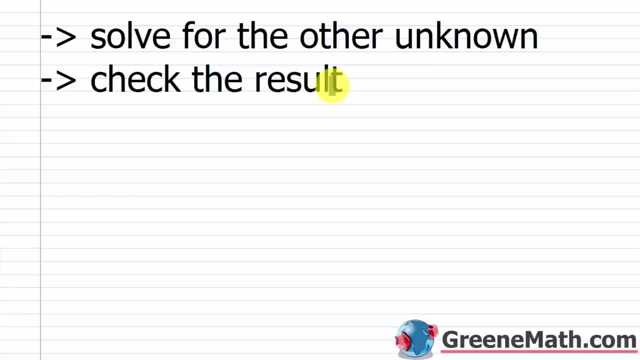 And then we just check our result. Remember, the solution has to work in both, All right. so let's take a look at another one. So we have negative 3x plus y equals 7.. We have negative 2x plus 2y equals 10.. So again, I'm looking for a variable that has a coefficient. 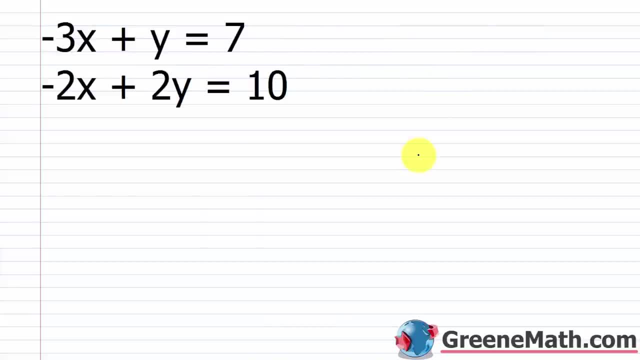 solution has to work in both all right so let's take a look at another one so we have negative 3x plus y equals 7 we have negative 2x plus 2y equals 10 so again I'm looking for a variable that has a coefficient of 1 or negative 1 if that exists sometimes it doesn't but in this case it does I have a coefficient of 1 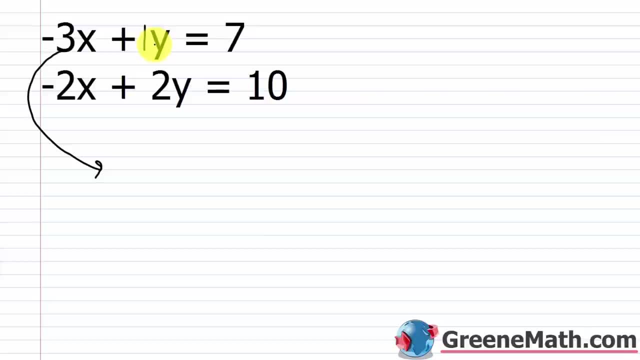 here so that means that this equation is really easy to solve for y I have negative 3x plus y equals 7 single step here just add 3x to both sides of the equation and I'm gonna get 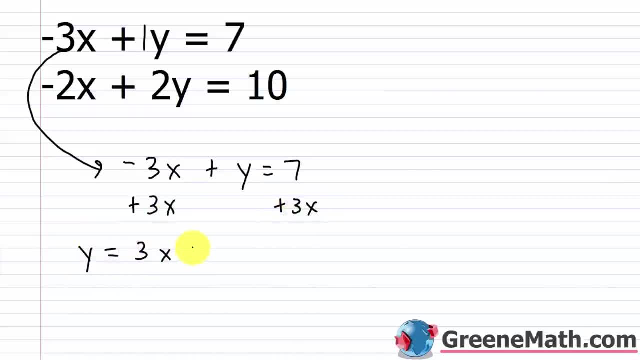 that y is equal to 3 X plus 7 now once I have that again I plug back in to the other equation so I used this equation to start so that means I'm gonna plug in for Y in this equation because I've solved 4y so I'm saying that Y is equal to or the same as 3 X plus 7 so I'm gonna plug this in, 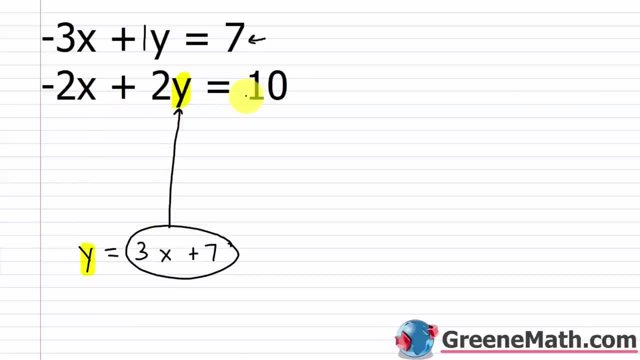 right here that way i have a linear equation in one variable and i can get a result for x so i'd have negative 2x plus 2 times y y is this quantity 3x plus 7. 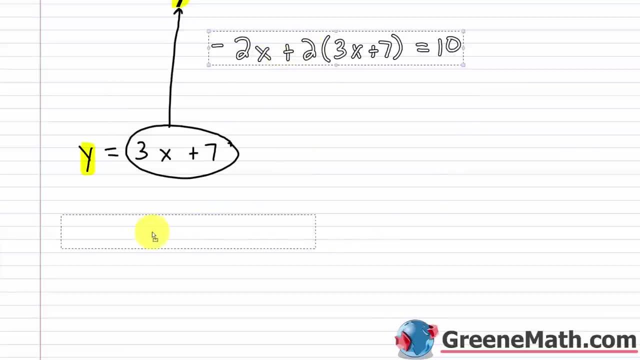 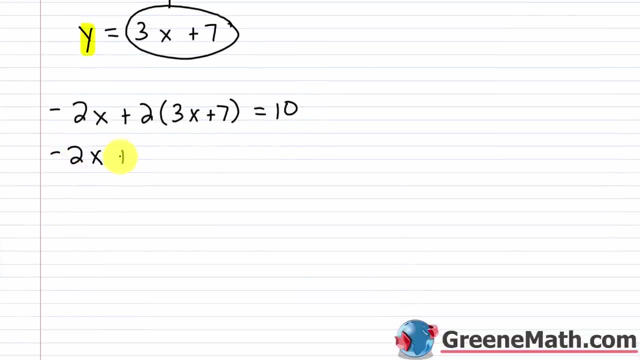 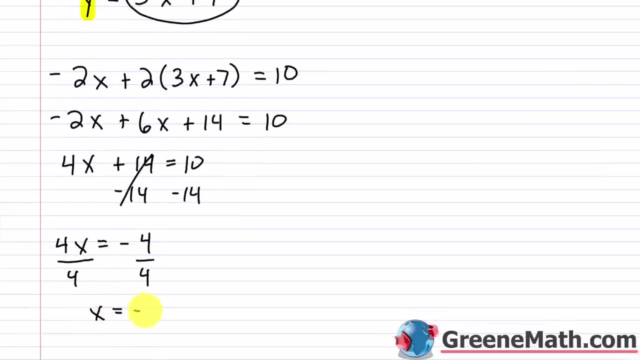 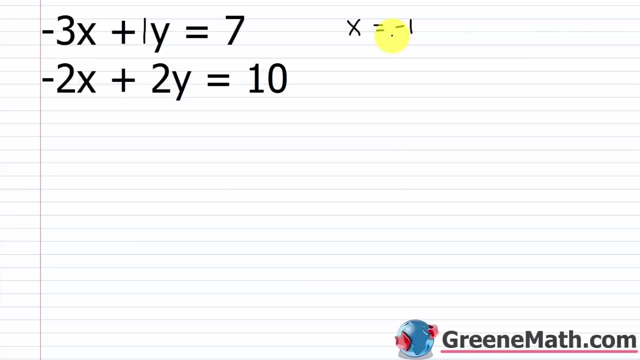 and this should be equal to 10. let me just drag this down here okay so we'd have negative 2x plus two times three x is six x and then two times seven is fourteen so plus fourteen this equals ten negative two x plus six x is four x so i have four x and then plus fourteen equals ten we would subtract fourteen away from each side of the equation that's gone i'll have 4x is equal to ten minus 14 is negative four divide both sides of the equation by 4, and we're going to get x is equal to negative 1. All right, so I know x equals negative 1, and now I can take that and I can plug it into either of the original equations. I can plug it in here or here, does not matter. So I'm going to plug it into the second one. So we have negative 2 times x is negative 1, so times negative 1, plus 2y equals 10. Negative 2 times negative 1 is 2, so that's positive 2, plus 2y equals 10. Subtract 2 away from each side of the equation. If that's gone, I'll have 2y is equal to 10 minus 2 is 8. 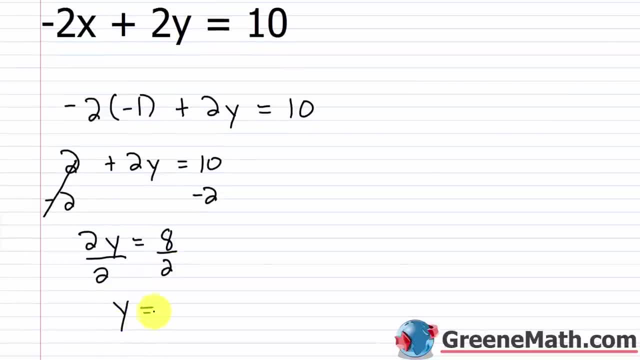 And then divide both sides of the equation by 2, and of course y is going to equal 4. 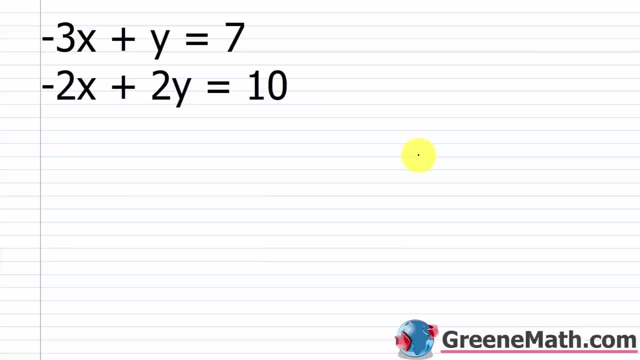 of 1 or negative 1, if that exists. Sometimes it doesn't, but in this case it does. I have a coefficient of 1 here, So that means that this equation is really easy to solve. for y I have negative. 3x plus y equals 7. Single step here. 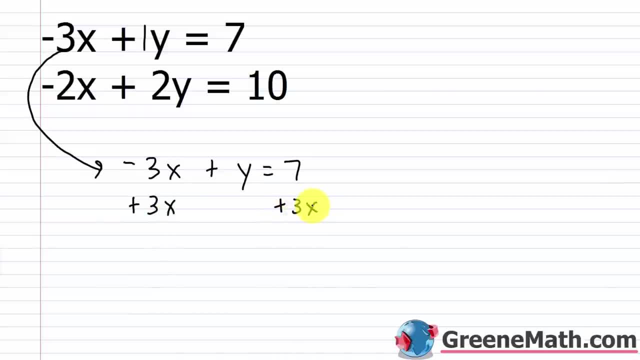 Just add 3x to both sides of the equation and I'm going to get that y is equal to 3x plus 7.. Now, once I have that again, I plug back in to the other equation. So I used this equation to 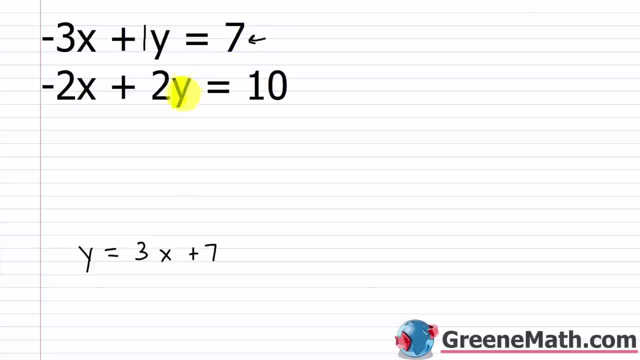 start. So that means I'm going to plug in for y in this equation, because I've solved for y. So I'm saying that y is equal to, or the same as, 3x plus 7.. So I'm going to plug this in. 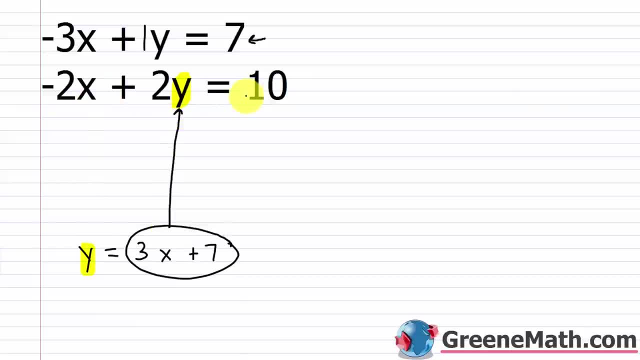 right here. That way I have a linear equation in one variable and I can get a result for x. So I'd have negative. 2x plus 2 times y, y is this quantity 3x plus 7. And this should be equal to 10.. Let me just drag this down here. 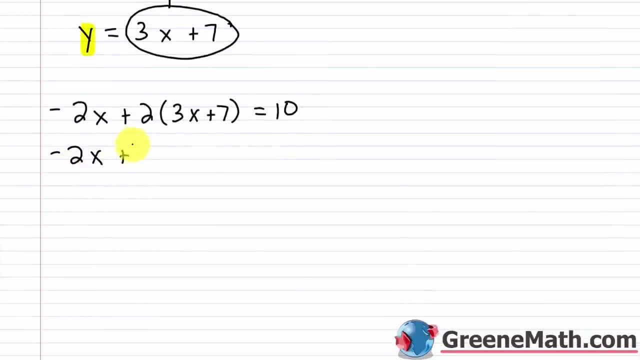 Okay, so we'd have negative 2x plus 2 times 3x is 6x, and then 2 times 7 is 14.. So plus 4x 14. This equals 10.. Negative 2x plus 6x is 4x. So I'd have 4x, And then plus 14 equals 10.. 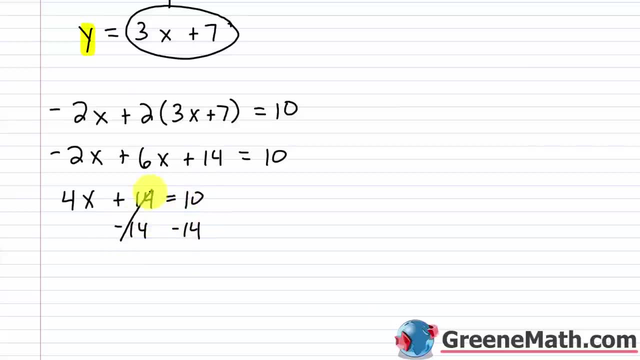 We would subtract 14 away from each side of the equation. That's gone. I'll have 4x is equal to 10 minus 14 is negative 4.. Divide both sides of the equation by 4, and we're going to get x is. 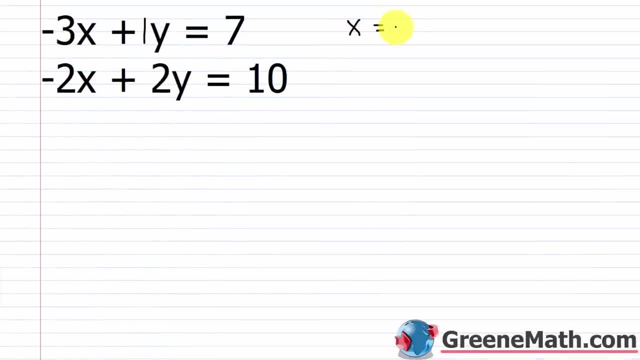 equal to negative 1.. All right, so I know x equals negative 1.. And now I can take that and I can plug it into either of the original equations. I can plug it in here or here, Does not matter. So I'm going to plug it into the second one. 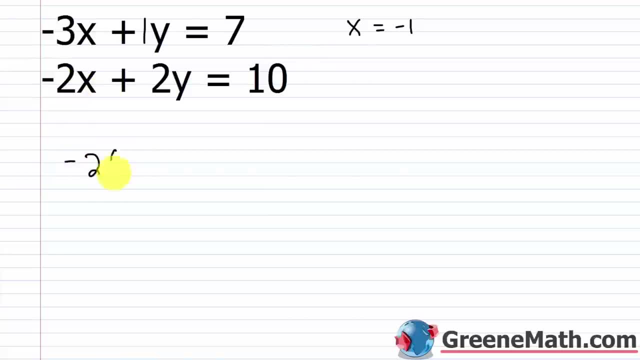 So we have negative 2 times x is negative 1.. So times negative 1 plus 2y equals 10.. Negative 2 times negative 1 is 2. So that's positive: 2 plus 2y equals 10.. Subtract 2 away from each side of: 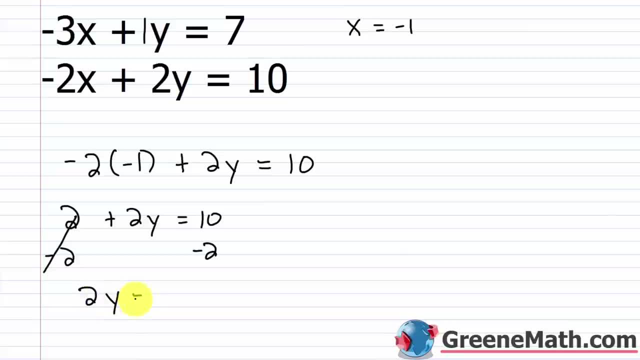 the equation That's gone I'll have: 2y is equal to 10 minus 2 is 8.. And then divide both sides of the equation by 2.. And, of course, y is equal to 10 minus 2 is 8.. And then divide both sides of the. 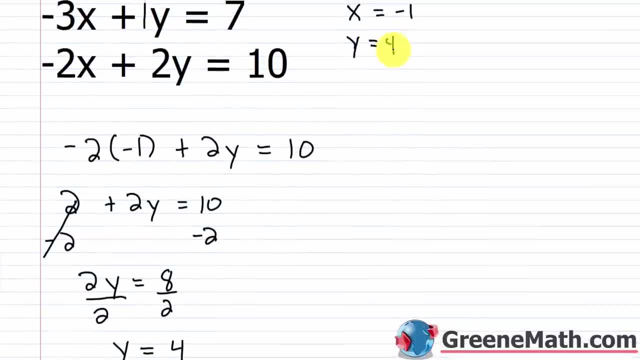 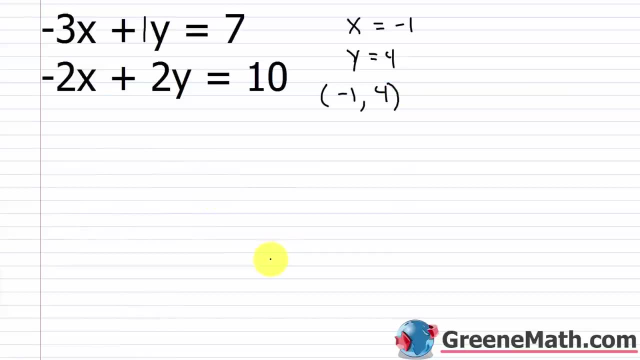 equation by 2. And of course y is going to equal 4.. So as an ordered pair, this is negative: 1 comma 4.. And of course you always want to check your work, So make sure this ordered pair is a solution. 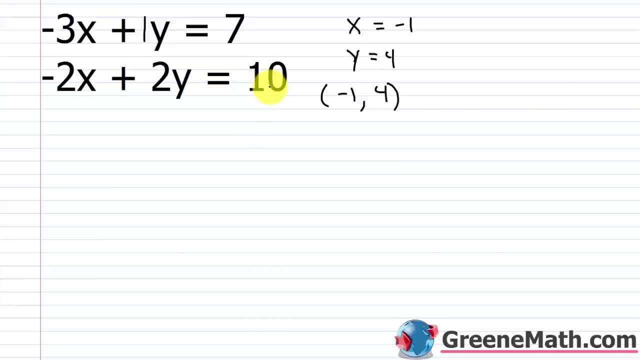 to this equation and to this equation. Remember, it's got to work in both to be a solution for the system. So we have negative 3 times x. x is negative 1.. So times negative 1 plus y, which is 4, equals 7.. 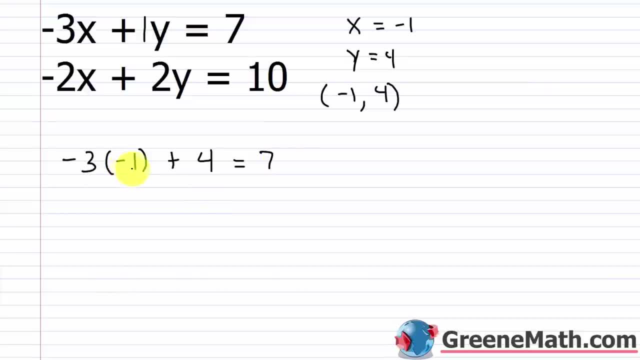 So you can follow that and see it's going to be true. Negative 3 times negative. 1 is 3.. 3 plus 4 is 7.. So that's going to check out. For the other one. we have negative 2x, So negative 2 times. 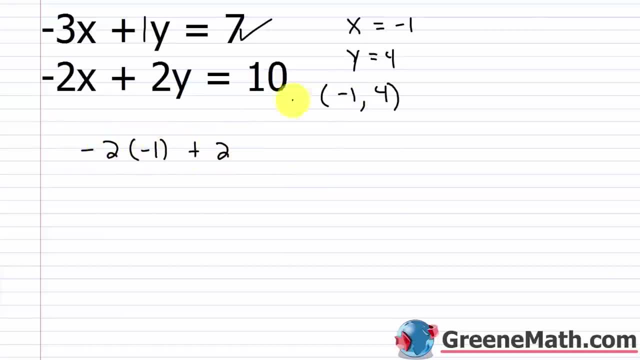 again negative 1 plus 2y. So for y we're plugging in a 4, equals 10.. So negative 2 times negative 1 is 2.. Plus 2 times 4 is 8. That should equal 10. And of course it does. So this result: 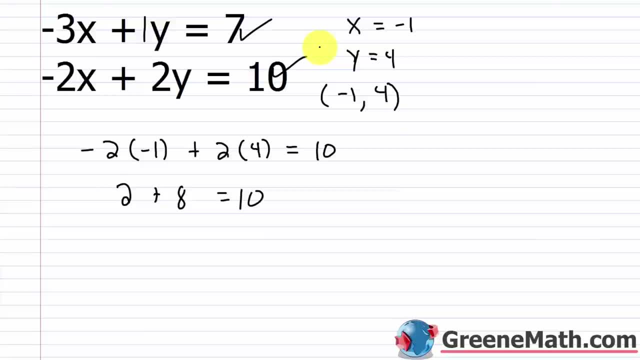 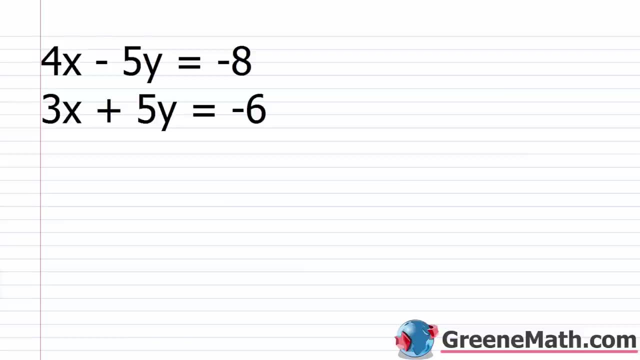 the ordered pair negative. 1 comma 4, is in fact the solution to each equation, And so it's a solution for our system. Well, let's take a look at another one. We have 4x minus 5y equals negative 8.. We have 3x plus 5y equals negative 6.. So again, I want to solve one. 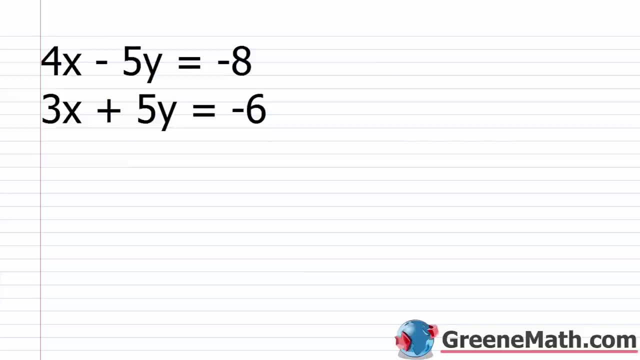 of the equations for one of the variables. Again, it doesn't matter which one. I like to look for a variable that has a coefficient of 1 or negative 1.. In this case we don't have that, So we might be better off using a different method, Another method we're going to learn in the next lesson. 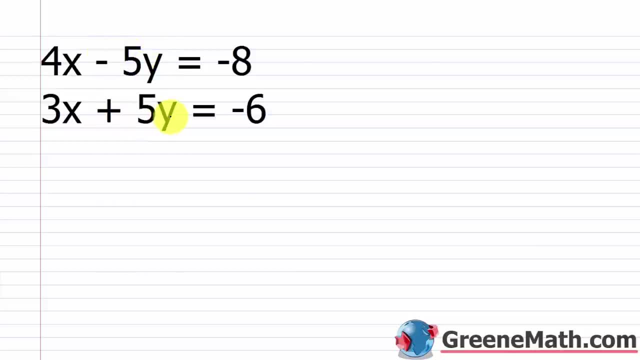 would be perfect here, because I have negative 5y and positive 5y And I know that probably doesn't make sense to you yet, but you'll see in the next lesson, For right now we're using substitution And it always works. It's just a little bit more work, So just solve one of these for one of the 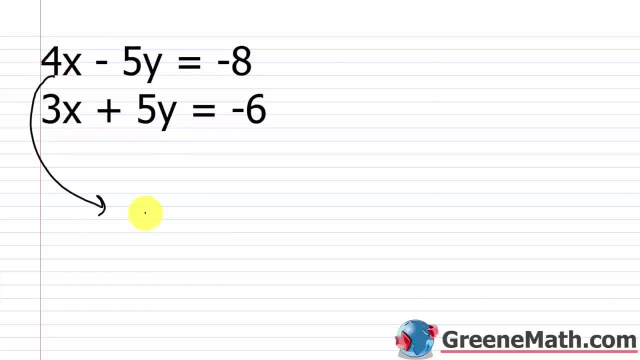 variables. So let's go ahead and just solve this first one for the variable x. So we have: 4x minus 5y equals negative 8. So I would add 5y to both sides of the equation. That's gone, We'll have. 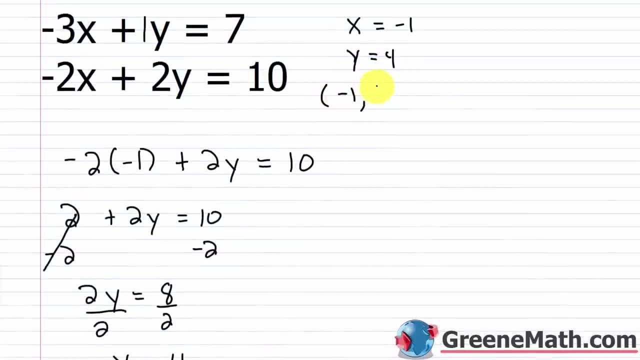 So as an ordered pair, this is negative 1 comma 4. And of course, you always want to check your work. So make sure this ordered pair is a solution to this equation and to this equation. Remember, it's got to work in both to be a solution for the system. So we have negative 3 times x, x is negative 1, so times 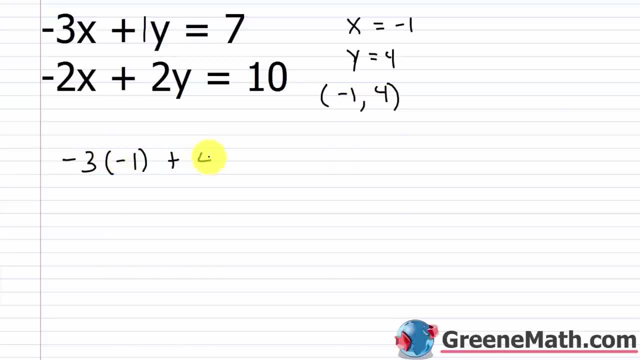 negative 1, plus y, which is 4, equals 7. You can eyeball that and see it's going to be true. 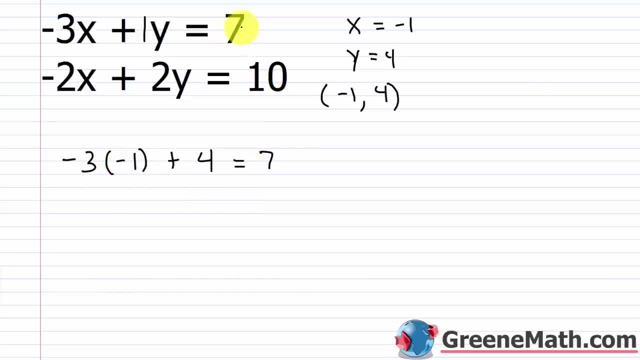 Negative 3 times negative 1 is 3, 3 plus 4 is 7, so that's going to check out. For the other one, we have negative 2x, so negative 2 times, again, negative 1, 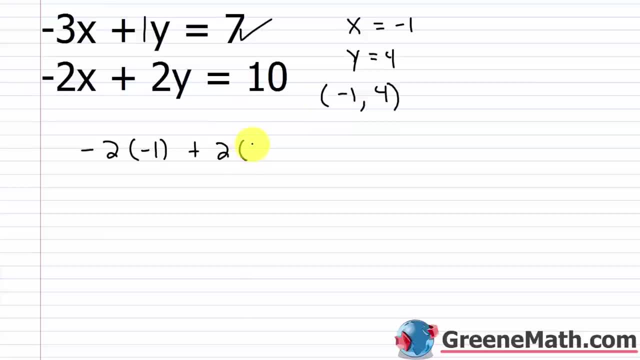 plus 2y, so for y, we're plugging in a 4, 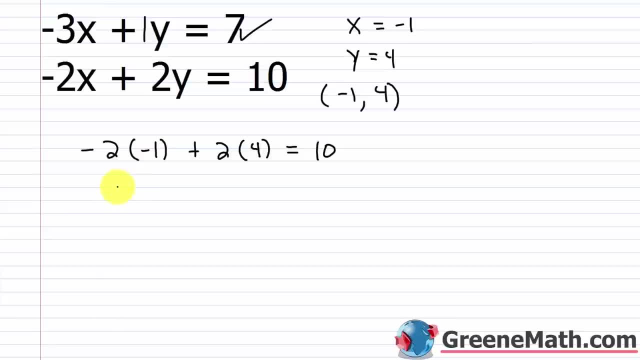 equals 10. So negative 2 times negative 1 is 2, plus 2 times 4 is 8, that should equal 10, and of course it does. 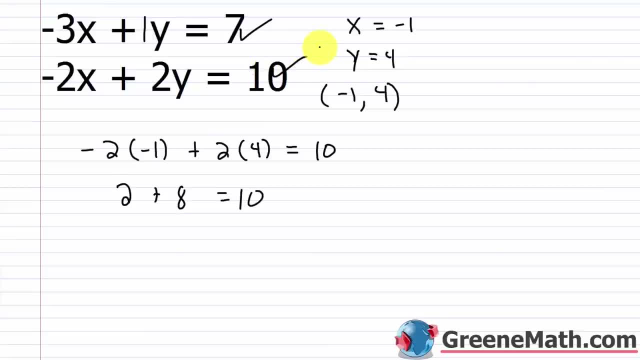 So this result, the ordered pair negative 1 comma 4, is in fact the solution to each equation, and so it's a solution for our system. 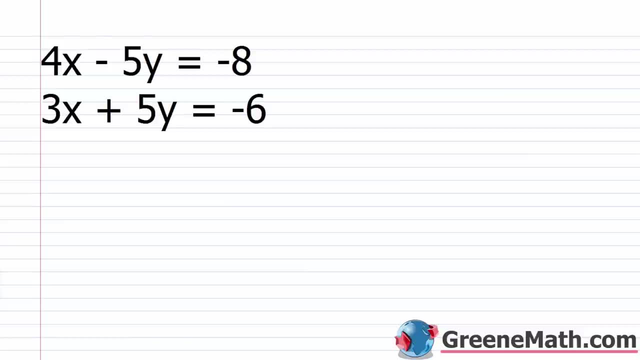 Alright, let's take a look at another one. We have 4x minus 5y equals negative 8. We have 3x plus 5y equals negative 6. So again, I want to solve one of the equations, for one of the variables. Again, it doesn't matter which one. I like to look for a variable that has a coefficient of 1, or negative 1. In this case, we don't have that, so 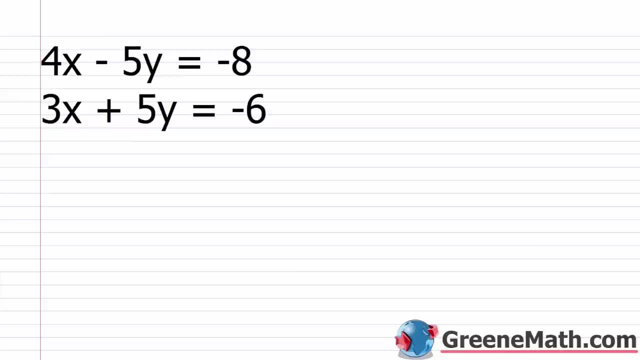 we might be better off using a different method. Another method we're going to learn in the next lesson is called elimination. 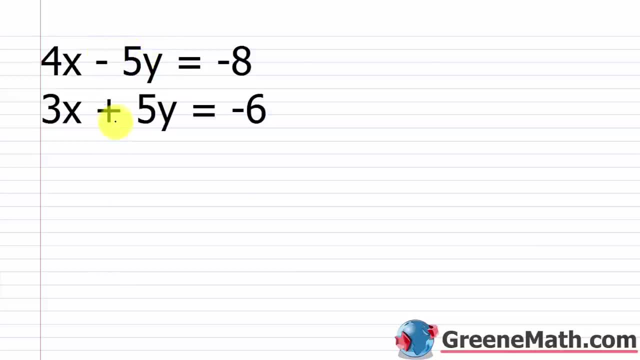 It would be perfect here, because I have negative 5y and positive 5y, and I know that probably doesn't make sense to you yet, but you'll see in the next lesson. For right now, 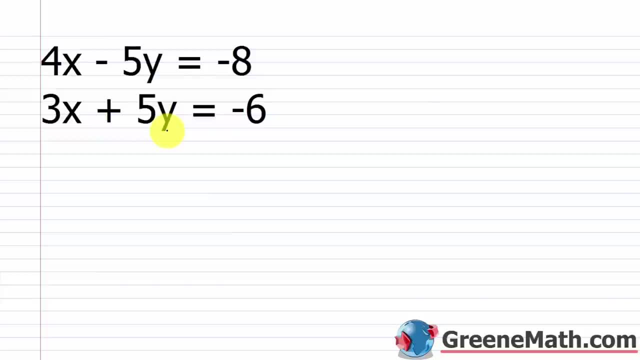 we're using substitution, and it always works. It's just a little bit more work, so just solve one of these for one of the variables. So let's go ahead and just solve this first one for the variable x. 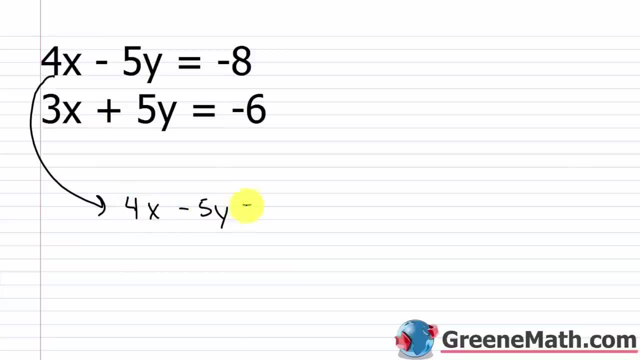 So we have 4x minus 5y equals negative 8. So I would add 5y to both sides of the equation. That's gone. We'll have 4x is equal to 5y minus 8, 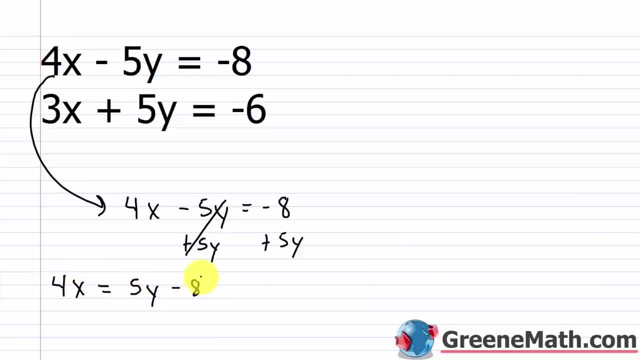 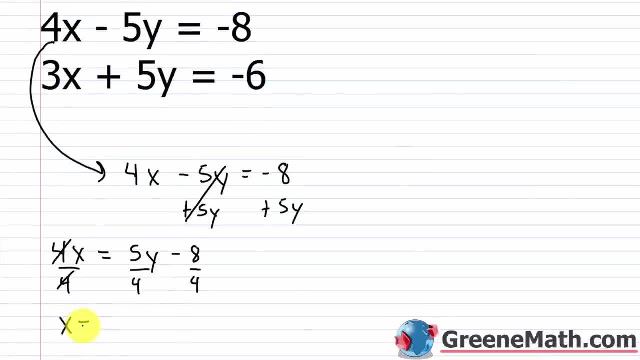 x is equal to 5y minus 8.. Then I'm going to divide both sides of the equation by 4.. That's going to cancel. I'll have: x is equal to 5 fourths y minus 8 over 4 is 2.. All right, So now I'm going to plug. 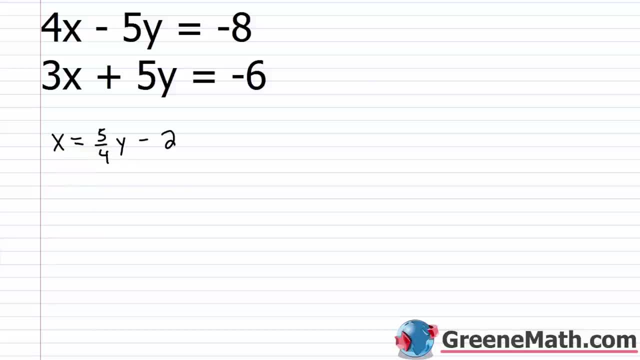 in 4x in the other equation. Again, it's got to be the other equation at this stage. So here's my x, And I'm saying x is equal to, or the same as, 5 fourths y minus 2.. So I'm just going to. 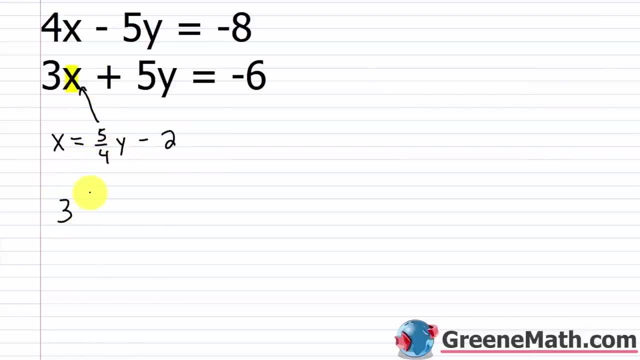 plug this in right there, So I'd have 3 times the quantity. Remember this is a quantity here: 5 fourths y minus 2.. Make sure you use parentheses. You don't want a silly mistake to cost you an answer on a test. So then, plus 5y equals negative 6.. 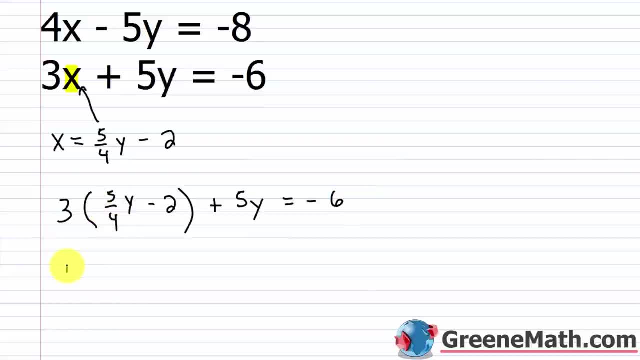 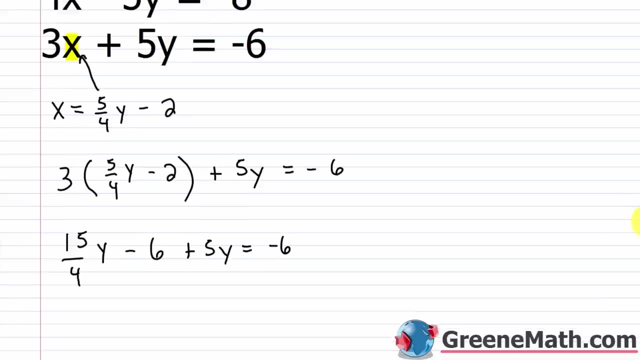 So 3 times 5 fourths would be 15. fourths times y minus 3 times 2. That's 6. Then plus 5y equals negative 6.. Let's go ahead and clear that denominator. Let's multiply both. 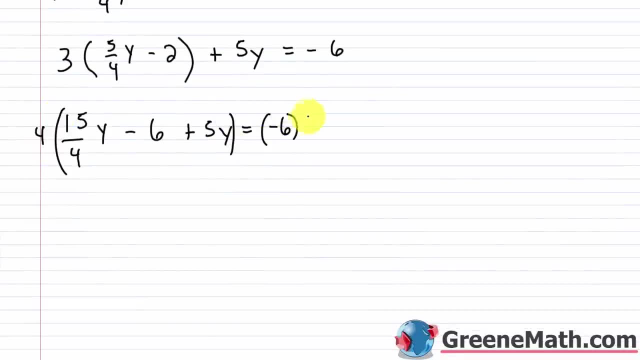 sides of the equation by 4.. So 4 times 15, fourths is obviously 15.. Then times y minus 4 times 6. That's 24.. Then plus 4 times 5y, That's 20y. And this equals negative 6 times 4.. That's negative. 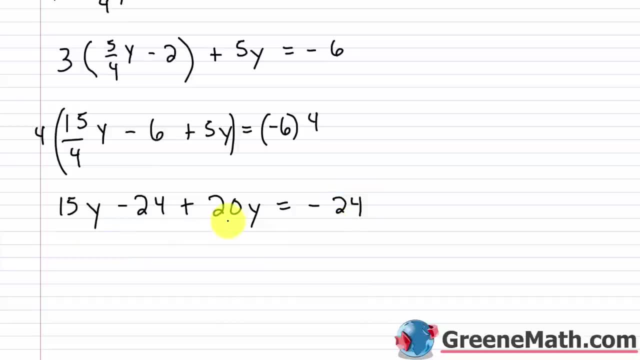 24.. All right, So 15.. 15y plus 20y is going to be 35y. Then minus 24 equals negative 24.. And what I've taught you before is that if you see the same thing on both sides of the equation, you can get rid of it Because of the addition. property of 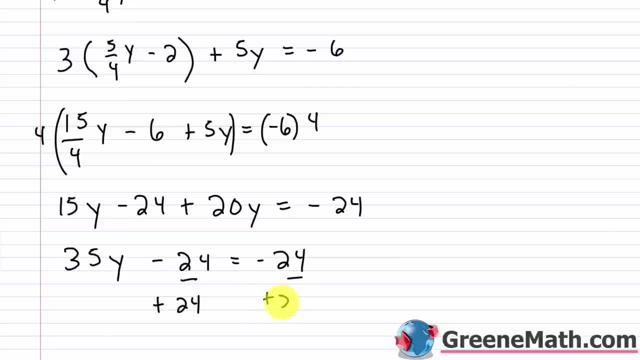 equality. if I add 24 to both sides of the equation, it's just going to go away. It's going to become 0.. So I'll have 35y on this side, And on the right side I'm just going to have 0.. 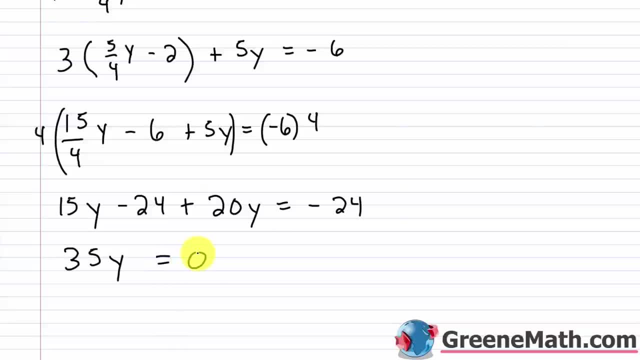 So this equals 0.. And obviously for 35y to equal 0, y has to be 0.. All right, I divide both sides by 35.. And y equals 0.. OK, So I know that y equals 0.. Now I just need to find a value for x And then I'm going to divide both sides of the equation by 4. 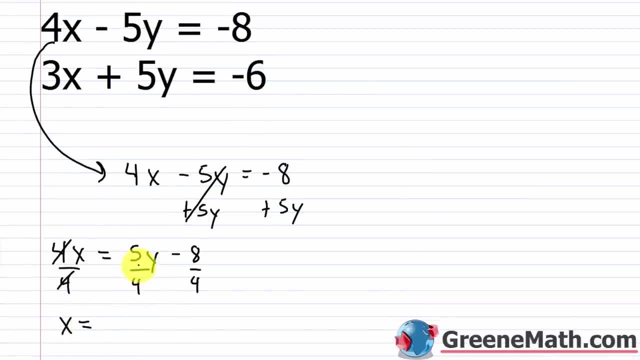 That's going to cancel. I'll have x is equal to 2. 5 fourths y minus 8 over 4 is 2. All right, so now I'm going to plug in 4x in the other equation. 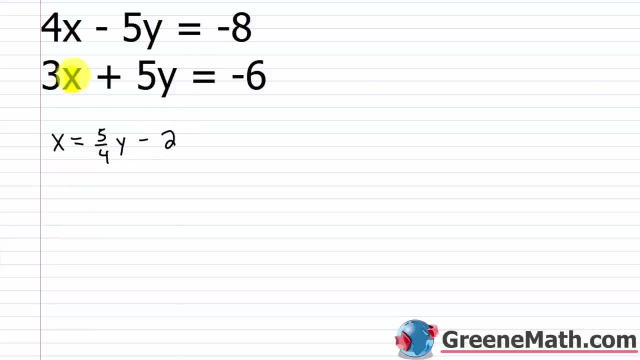 Again, it's got to be the other equation at this stage. So here's my x, and I'm saying x is equal to or the same as 5 fourths y minus 2. So I'm just going to plug this in right there. So I'd have 3 times the quantity. Remember, this is a quantity here. 5 fourths y minus 2. Make sure you use parentheses. You don't want a silly mistake to cost you an answer on a test. So then plus 5y equals negative 6. So 3 times 5 fourths would be 15 fourths times y minus 3 times 2. That's 6. 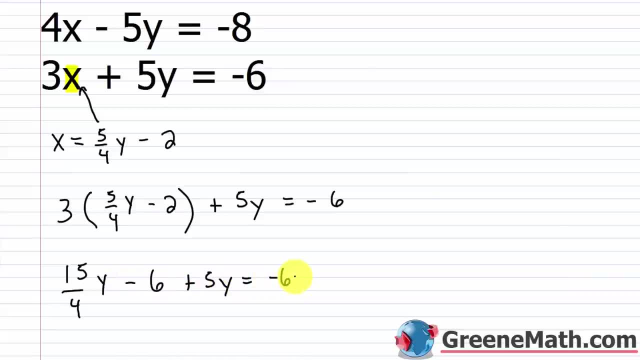 Then plus 5y equals negative 6. Let's go ahead and clear that denominator. Let's multiply both sides of the equation by 4. 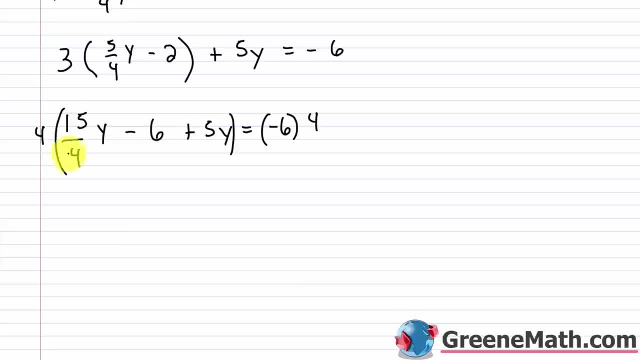 So 4 times 15 fourths is obviously 15. Then times y minus 4 times 6, that's 24. Then plus 4 times 5y, that's 20y. This equals negative 6 times 4, that's negative 24. 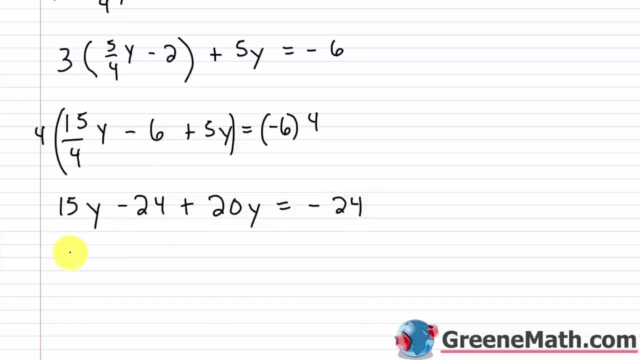 All right, so 15y plus 20y is going to be 35y. Then minus 24 equals negative 24. 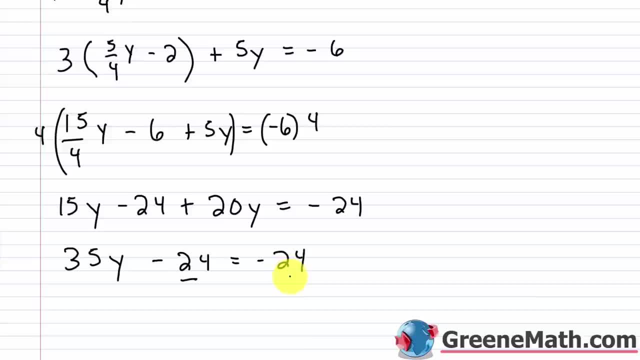 And what I've taught you before is that if you see a square, you're going to have a square on both sides of the equation, you can get rid of it. Because of the addition property of equality, if I add 24 to both sides of the equation, it's just going to go away. It's just going to become 0. So I'll have 35y on this side. And on the right side, I'm just going to have 0. So this 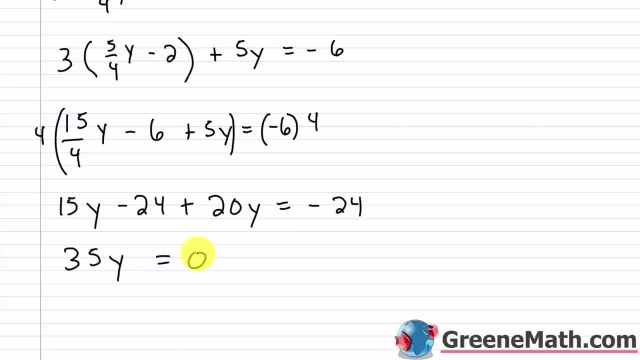 equals 0. And obviously, for 35y to equal 0, y has to be 0. I'd divide both sides by 35. And y, 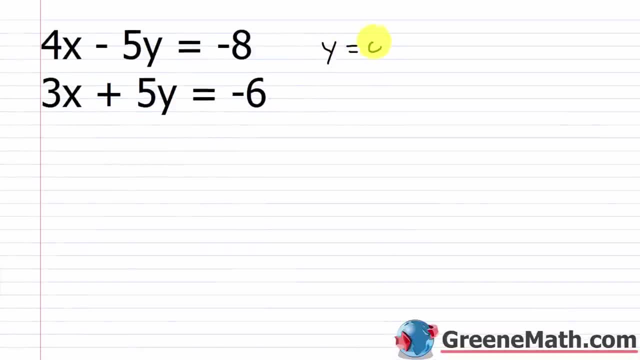 y equals 0. Okay, so I know that y equals 0. Now I just need to find a value for x. And again, I can use either equation and substitute a 0 in for y, solve for x. So let's go ahead and use the second equation. So we'd have 3x plus 5 times 0 equals negative 6. And so 5 times 0 is 0, so that's gone. I'd have 3x is equal to negative 6. Divide both sides by 3. And you get x is equal to negative 2. So this ordered pair would be negative 2 comma 0. All right, so again, the last thing we want to do 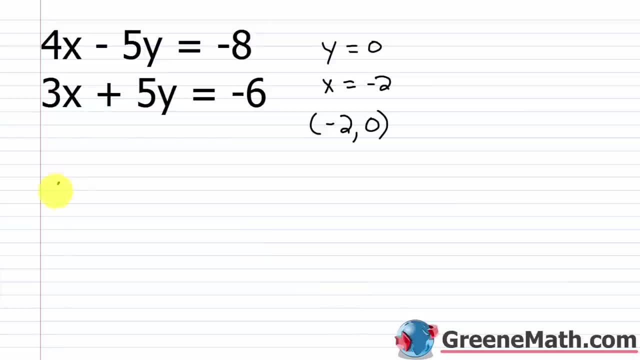 is just check our work, make sure we got the right answer. So we have 4 times, for x, I'm plugging in a negative 2, minus 5 times 0 equals negative 8. And that's true. 4 times negative 2 is negative 8. So 5 times 0 is 0. And so we have minus 0 there. So it's basically just negative 8 is going to be equal to negative 8. So this one is true. So then the next one, we have 3x. So 3 times 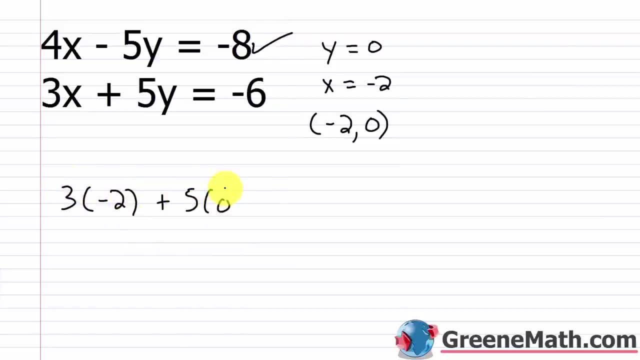 negative 2 plus 5y, 5 times 0, equals negative 6. So 3 times negative 2 is negative 6. Then plus 5 times 0 is 0. So plus 0, I can just kind of get rid of that. So negative 6 equals negative 6. 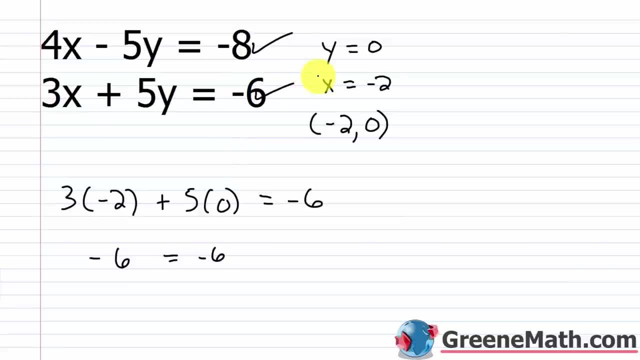 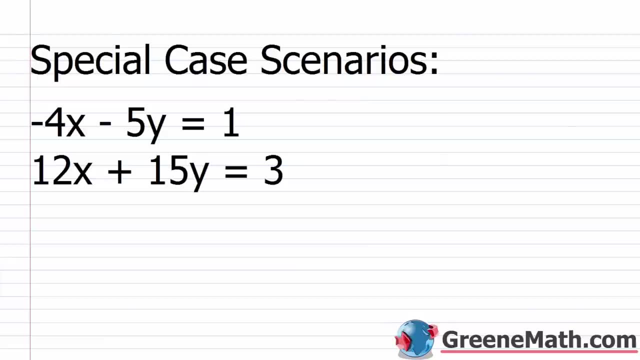 So this one works out as well. So negative 2 comma 0, that ordered pair, is a solution for our system. So all in all, not a very difficult procedure to execute. You just have to remember what to do in what order, right? I mean, you're basically just going to end up solving a linear 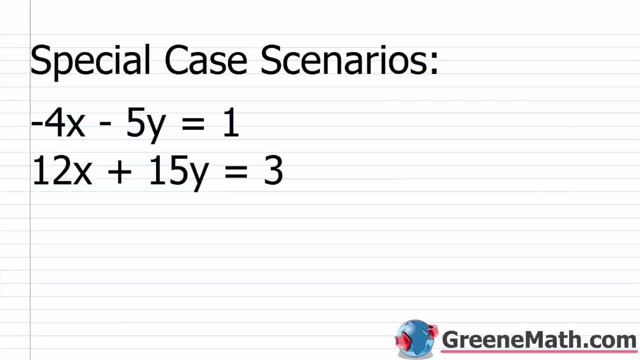 table to get your value for x and to get your value for y. So nothing that's too difficult. 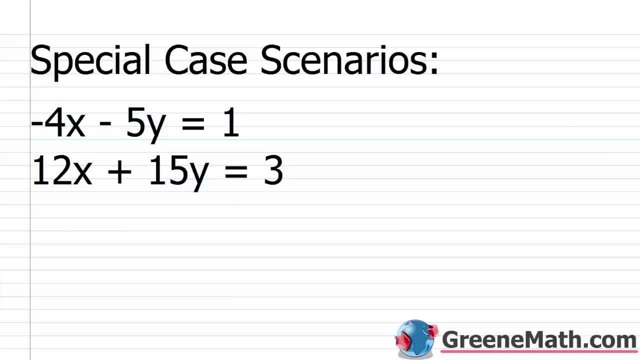 All right, let's talk a little bit about special case scenarios. So you'll recall when we did our lesson on graphing that we looked at two special cases. One special case was that we had parallel lines, right? So we had a system that would never have a solution because the two lines would never 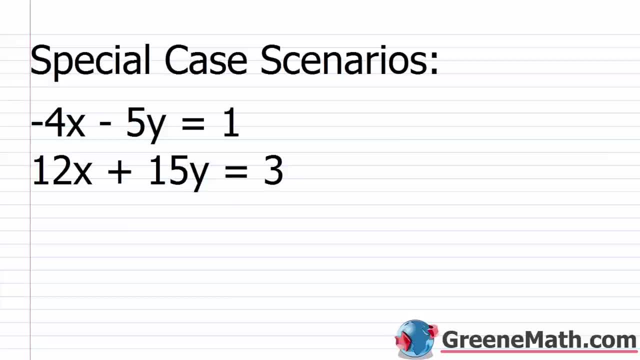 ever cross. So there would be no ordered pair that would satisfy both. Then you also have a special case scenario where you have a system that would never have a solution because the two lines you have the exact same line, right? So one line was manipulated to look like it was different, 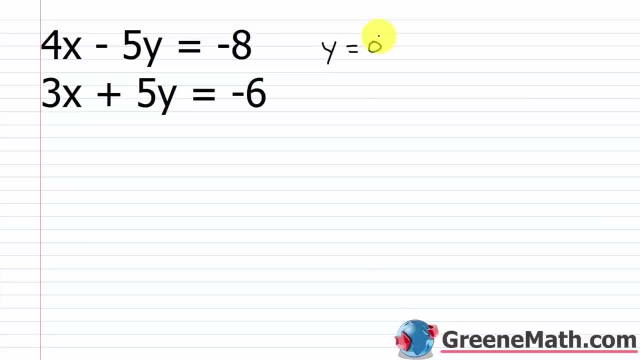 again, I can use either equation and substitute a 0 in for y, solve for x. So let's go ahead and use the second equation. So we'd have 3x plus 5 times 0 equals negative 6. And so 5 times. 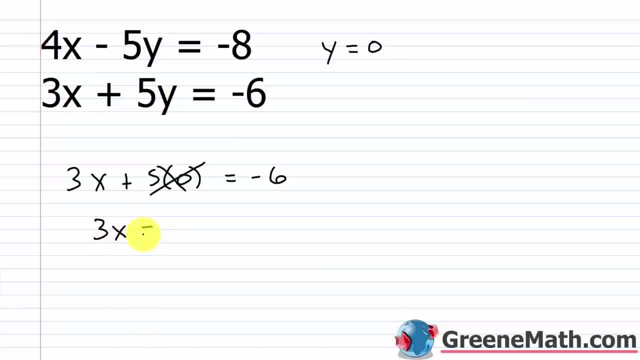 0 is 0. So that's gone. I'd have: 3x is equal to negative 6. Divide both sides by 3. And you get x is equal to negative 2. So this ordered pair would be negative. 2 comma 0.. All right, So again. 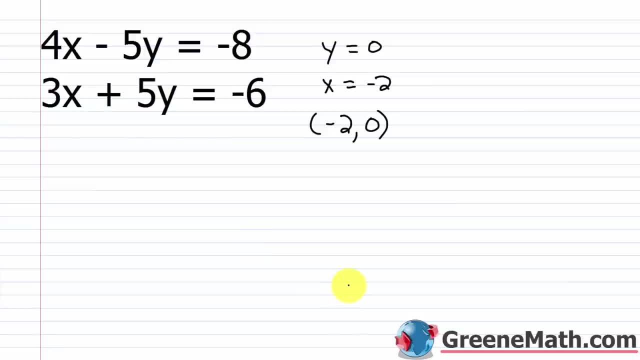 the last thing we want to do is just check our work, make sure we got the right answer. So we have 4 times for x- I'm plugging in a negative 2, minus 5 times 0 equals negative 8.. 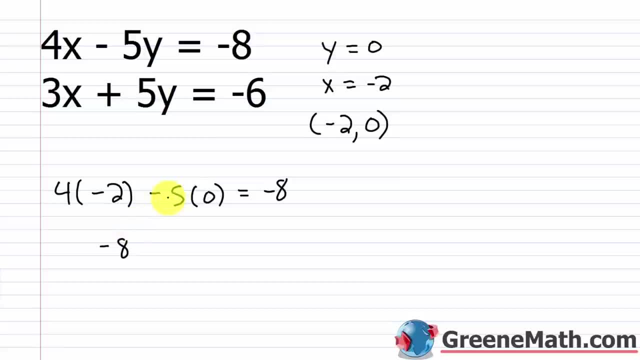 And that's true. 4 times negative 2 is negative 8.. So 5 times 0 is 0. And so we have minus 0 there. So it's basically just negative. 8 is going to be equal to negative 8.. So this one is true. So then the next one: we have 3x, So 3 times negative 2. 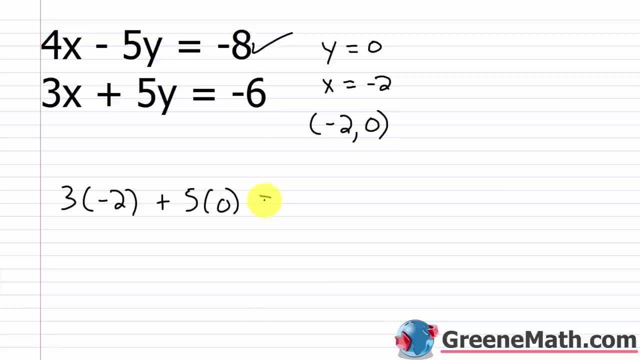 plus 5y 5 times 0, equals negative 6. So 3 times negative 2 is negative 6. Then plus 5 times 0 is 0. So plus 0, I can just kind of get rid of that. 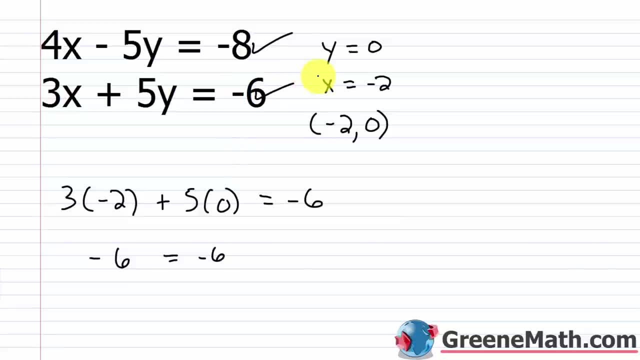 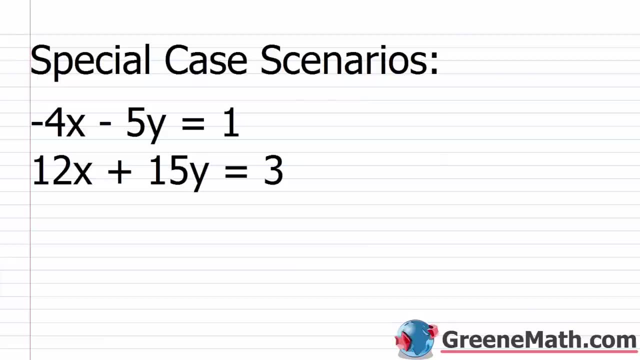 So negative 6 equals negative 6. So this one works out as well. So negative 2 comma 0, that ordered pair is a solution For our system. So, all in all, not a very difficult procedure to execute. You just have to remember what to do and what order, right? I mean, you're basically just going. 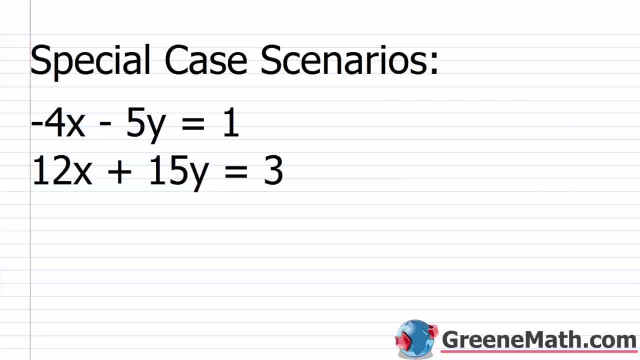 to end up solving a linear equation and one variable to get your value for x and to get your value for y. So nothing that's too difficult. All right, Let's talk a little bit about special case scenarios. So you'll recall when we did our lesson on graphing that we looked at two special 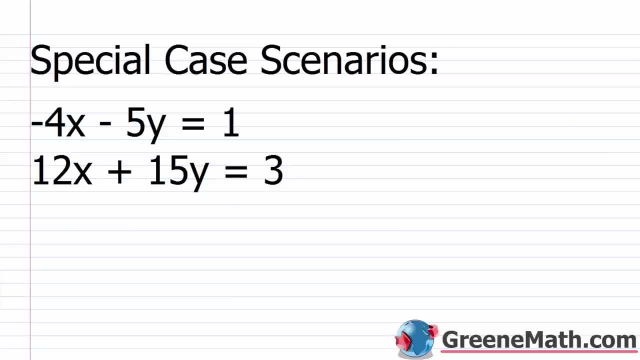 cases. One special case was that we had parallel lines right, So we had a system that would never ever have a solution because the two lines would never ever cross, So there would be no ordered pair that would satisfy both. Then you also have a special case scenario where you have the exact 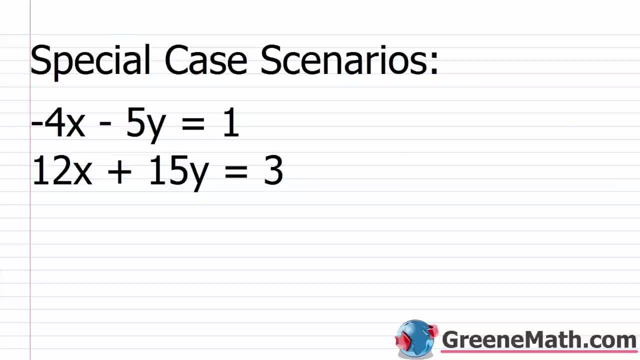 same line, right? So one line was manipulated to look like it was different, but it was the same, And so you had an infinite number of solutions. Now, when you have a special case scenario with no solution, you're going to end up with a nonsensical statement like I don't know. 4 equals. 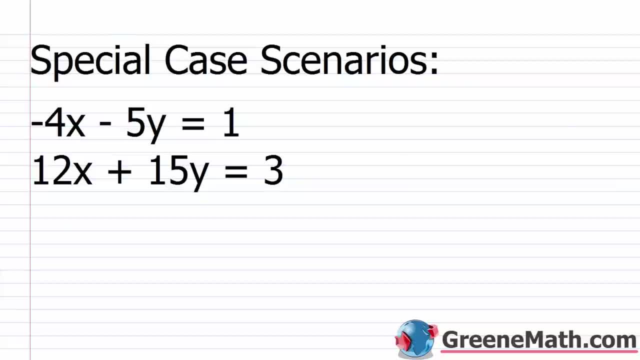 but it was the same. And so you had an infinite number of solutions. Now, when you have a special case scenario with no solution, you're going to end up with a nonsensical statement like, I don't know, 4 equals 12 or 0 equals negative 36. The two sides won't be equal, but you'll 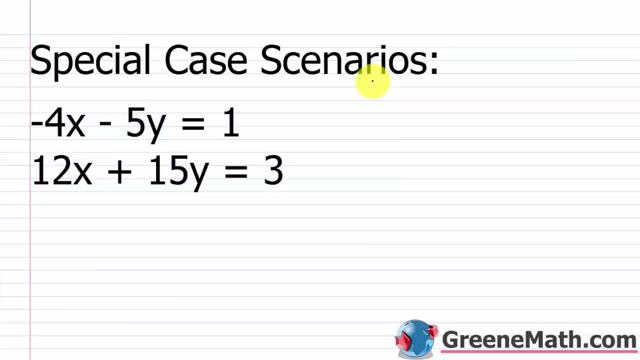 have an equal assignment. So let me show you with this example. We have negative 4, x minus 5, y equals 1. We have 12, x plus 15, y equals 3. So let me solve this first equation for 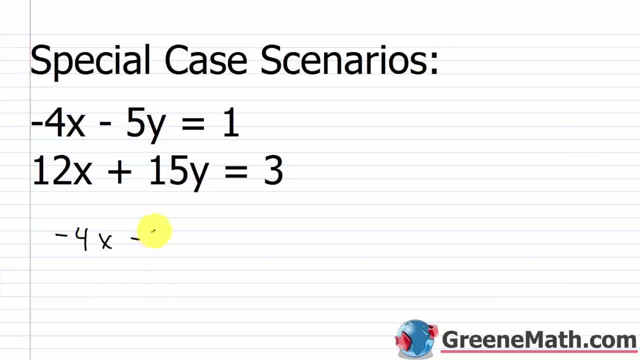 y. So we have negative 4, x minus 5, y equals 1. I'll add 4, x to both sides of the equation. 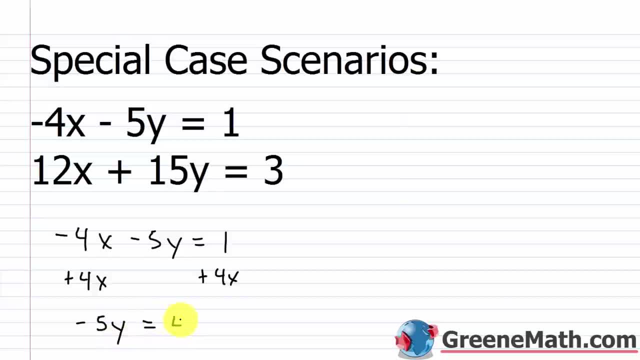 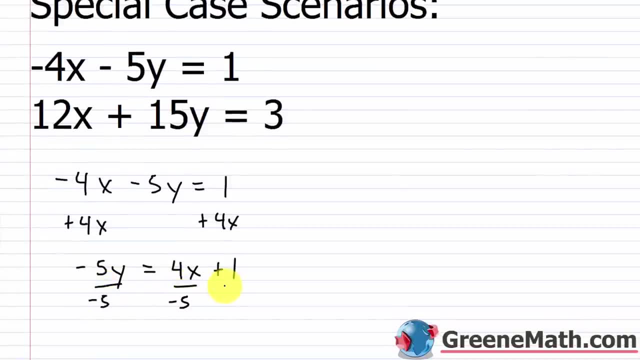 And I'll have negative 5, y is equal to 4, x plus 1. Now I want to divide both sides of the equation by negative 5. And so what I'd have is, y equals 4 over negative 5, that's just negative 4 fifths, then times x. And then minus, we have 1 over negative 5. So I put minus, and then 1 fifth. So that's solved for y. 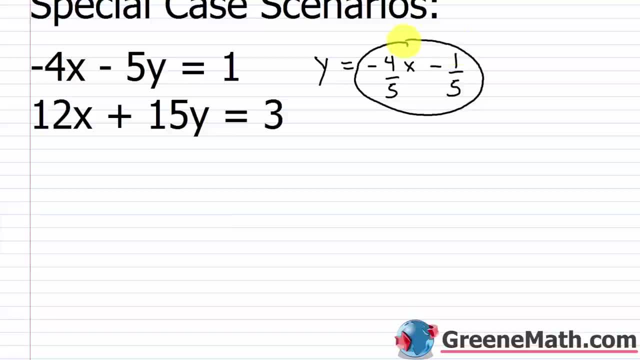 And now we can plug in for y in the other equation. So remember, y is equal to or the same as negative 4 fifths x minus 1 fifth. So I'm going to plug in for y here. And again, what I'm plugging in has only an x variable. So I'm going to plug in for y here. And again, what I'm plugging in has only an x variable. So I'm going to plug in for y here. And again, what I'm plugging in has only an x variable. 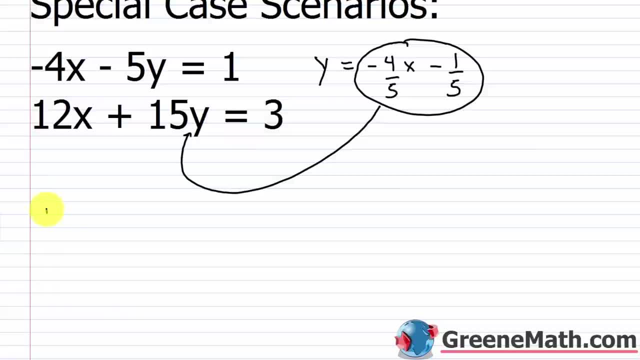 So I'd have a linear equation of one variable now. So 12x plus 15 times, again, you've got to use parentheses here, because this is a quantity. So negative 4x over 5, or negative 4 fifths x, if you want to say it that way, minus 1 fifth. Okay, and this is going to be equal to 3. 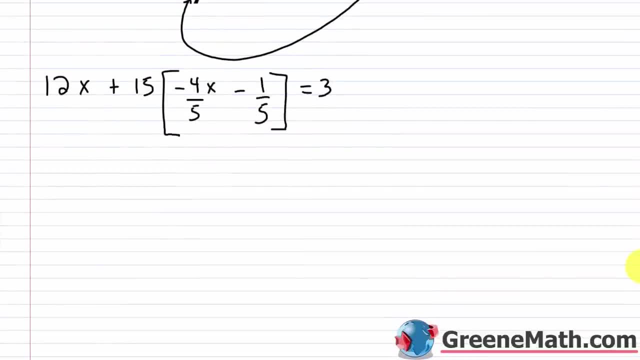 So unfortunately, when we go through and solve this, we're going to get some nonsense. So we'll have 12x, 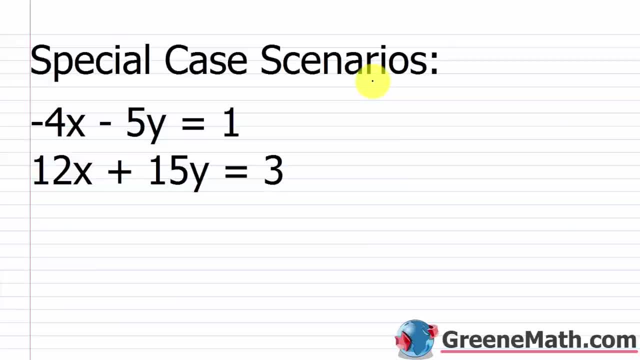 12. Or 0 equals negative 36. The two sides won't be equal, but you'll have an equal sign there. So let me show you with this example: We have negative. 4x minus 5y equals 1.. We have 12x plus. 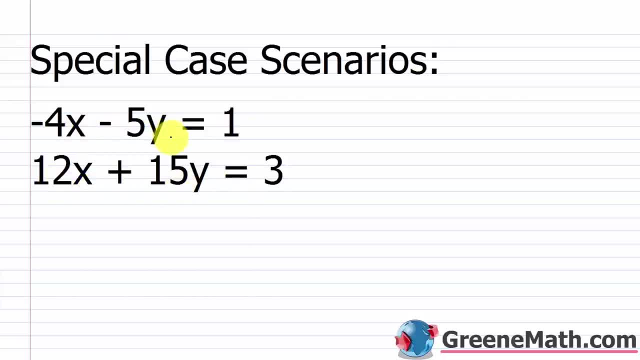 15y equals 3.. So let me solve this first equation for y. So we have negative. 4x minus 5y equals 1.. I'll add 4x to both sides of the equation And I'll have negative. 5y is equal to 4x. 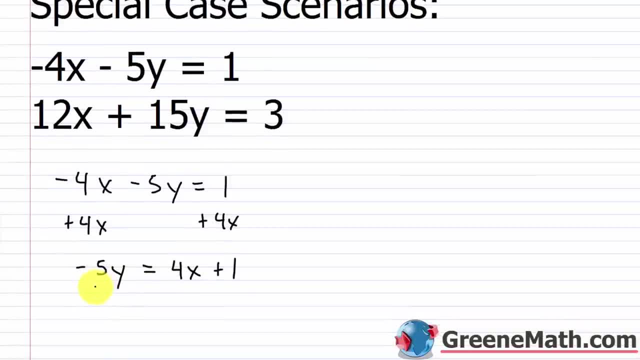 Plus 1.. Now I want to divide both sides of the equation by negative 5.. And so what I'd have is y equals 4 over negative 5. That's just negative 4 fifths. Then times x And then minus, we have 1 over negative 5.. So I put minus and then 1 fifth. 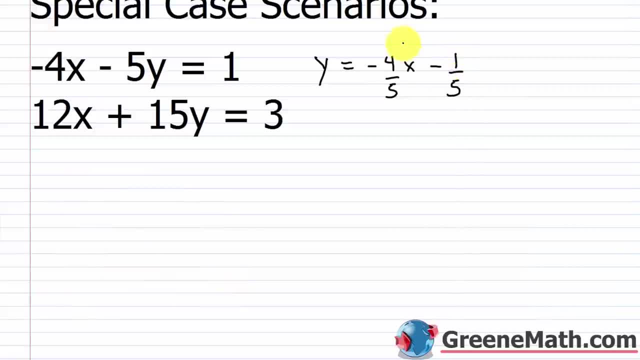 So that's solved for y, And now we can plug in for y in the other equations. So remember, y is equal to, or the same as, negative 4 fifths x minus 1 fifths. So I'm going to plug in for y here. And again, what I'm plugging in has only an x variable, So I'd 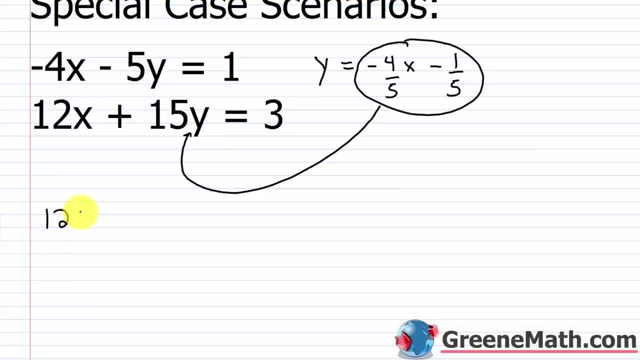 have a linear equation of one variable now, So 12x plus 15 times- again, you've got to use parentheses here because this is a quantity, So negative 4x over 5, or negative 4 fifths x, if you want to say it that way, minus 1 fifth. Okay. 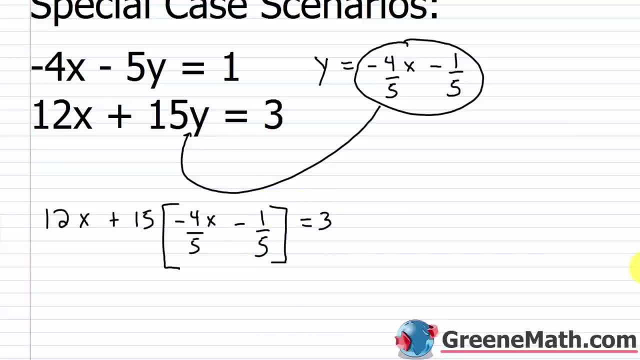 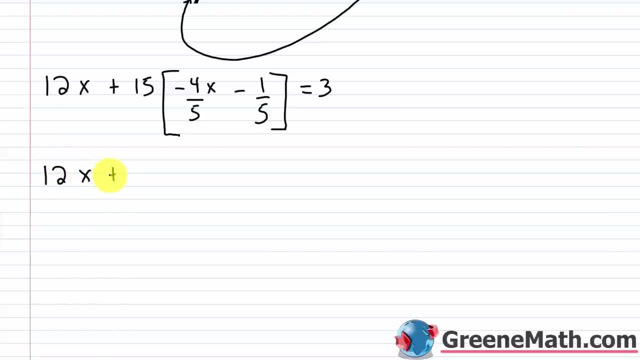 And this is going to be equal to 3.. So unfortunately, when we go through and solve this, we're going to get some nonsense. So we'll have 12x plus 15 times negative 4 fifths. The 15 would cancel. 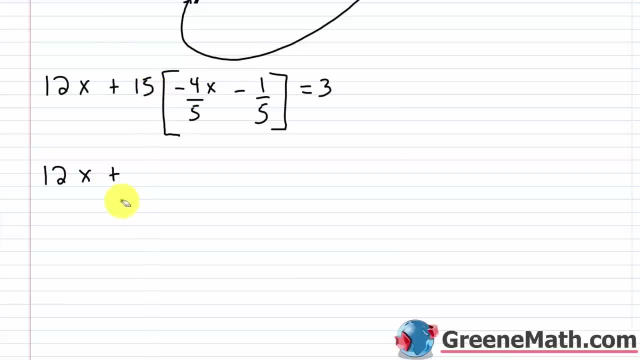 with the 5 and give me 3.. 3 times negative 4 is negative 12.. So I might as well just put minus 12x And then 15 times negative 1. fifth, The 15 would cancel with the 5 and 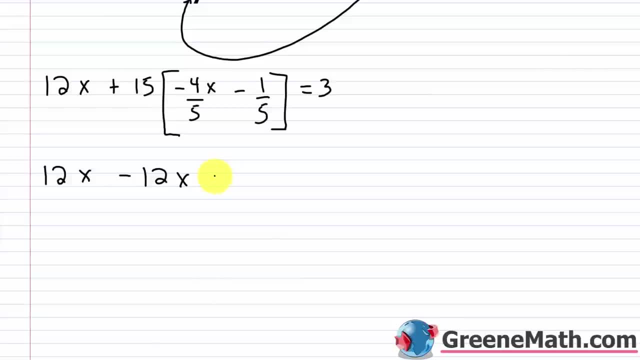 give me a 3.. 3 times negative 1 is negative 3. So minus 3.. So you can see if you combine like terms here, 12x minus 12x is zero. So I'd end up with this canceling and me having negative. 3 equals 3, which is false. So if you get something like this: 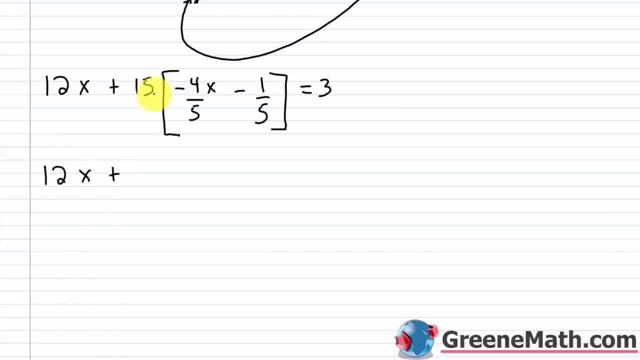 plus 15 times negative 4 fifths. The 15 would cancel with a 5 and give me 3. 3 times negative 4 is negative 12. So I might as well just put minus 12x, and then 15 times negative 1 fifth. The 15 would cancel with a 5 and give me a 3. 3 times negative 1 is negative 3. So minus 3 equals 3. So you can see if you combine like terms here, 12x minus 12x is 0. So I'd end up with this canceling, and me having negative 3, equals 3, which is false. So if you get something like this, don't freak out. You have a system that 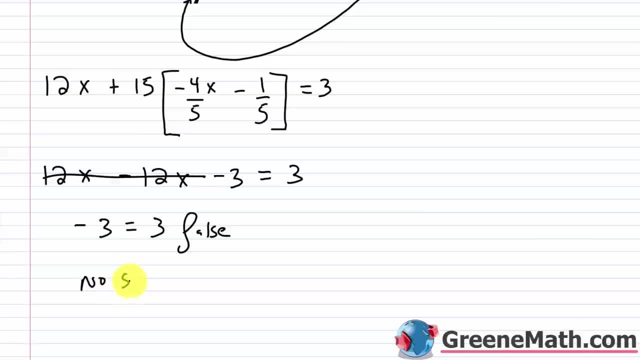 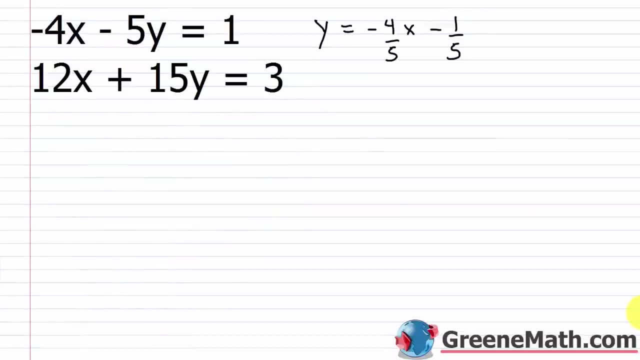 has no solution. You have a no solution. And that's how you can tell. You get a nonsensical statement like that. Negative 3 equals 3, right? That's clearly false. All right, so to kind of 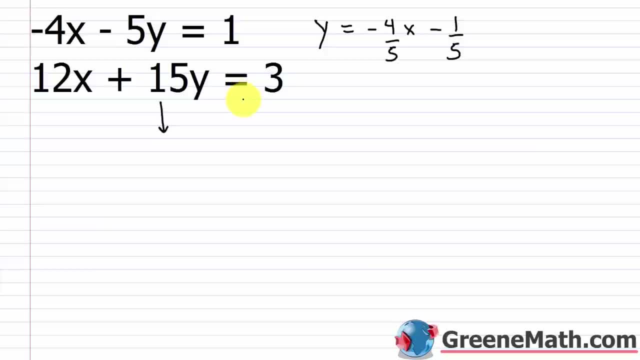 prove that this has no solution, I want to also solve this equation for y, and show you that you have the same slope, but a different y-intercept. So we'd have 12x plus 15, 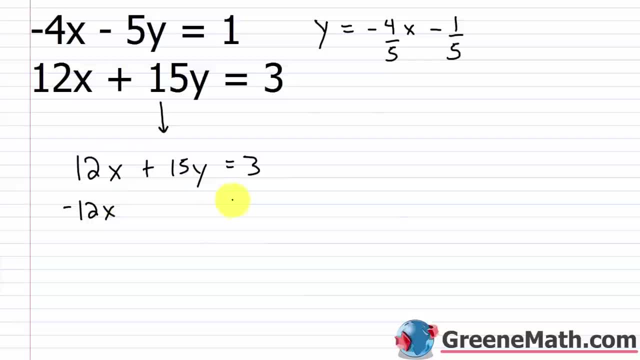 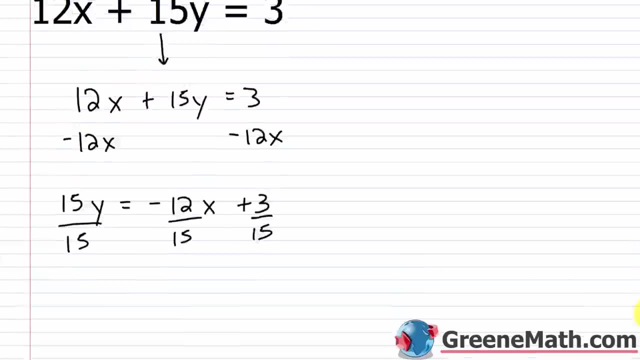 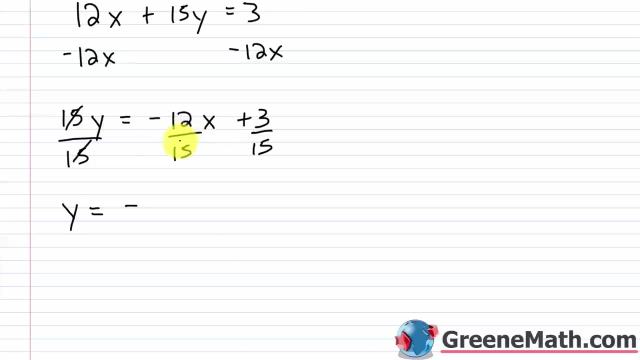 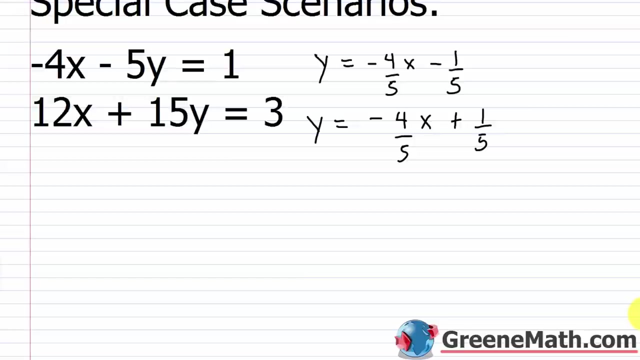 y equals 3. We're going to subtract 12x away from each side of the equation. We're going to have 15y is equal to negative 12x plus 3. Divide both sides of the equation by 15. And what are we going to have? This cancels. I'll have y is equal to negative 12 is divisible by 3, and so is 15. So negative 4 fifths times x plus 3 fifteenths. Each is divisible by 3. So I'll have 1 fifth. So it's really easy to make a mistake here and think that you have the exact same equation, but you don't. And what's different here is a 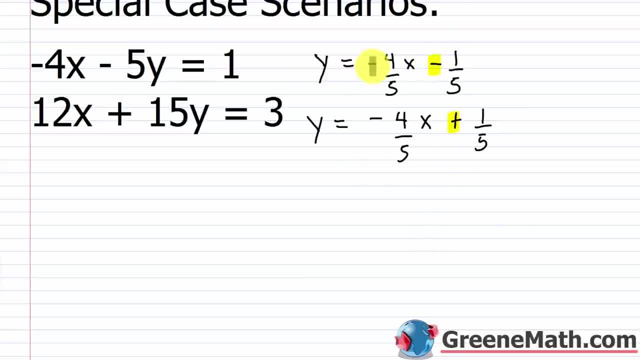 minus and a plus. So you have y equals negative 4 fifths x minus 1 fifth. So the y-intercept occurs at 0 comma negative 1 fifth. For this one, we have y equals negative 4 fifths x plus. Okay, see how that's different? This is a minus, this is a plus, one-fifth. So the y-intercept occurs here at zero comma one-fifth. So they're very similar, but they're not the same equation. And so this is not a scenario where we have an infinite number of solutions. We don't have a solution at all. So these two equations will never cross on the 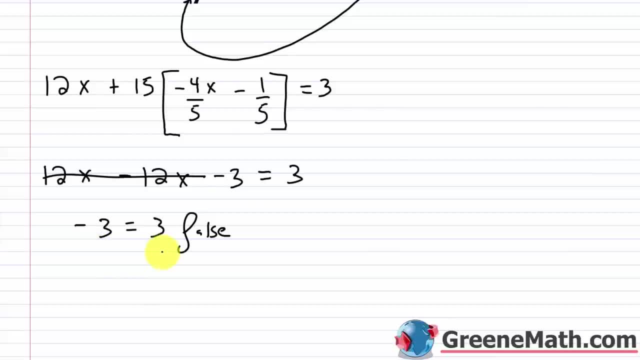 don't freak out. You have a system that has no solution. You have a new solution And that's how you can tell. You get a nonsensical statement like that: Negative 3 equals 3, right, That's clearly false. All right, So to kind of prove that this has no solution. 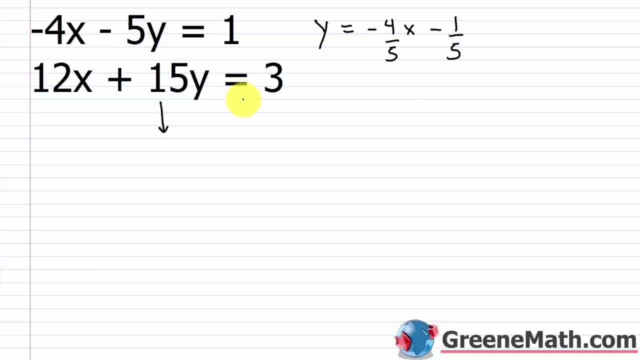 I want to also solve this equation for y and show you that you have the same slope but a different y-intercept. So we'd have 12x plus 15y equals 3.. We're going to subtract 12x away from each side of the equation. We're going to have 15y is equal to negative 12x. 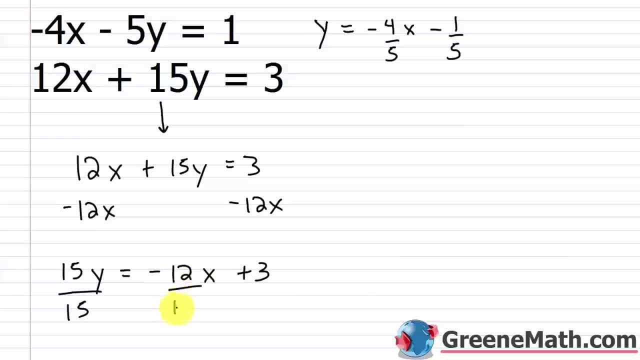 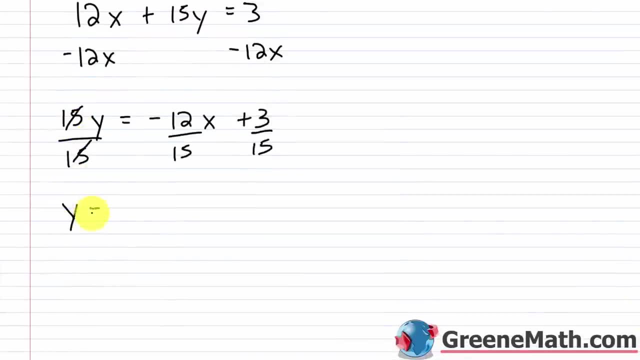 plus 3.. Divide both sides of the equation by 15.. And what are we going to have? This cancels, We'll have. y is equal to negative, 12 is divisible by 3, and so is 15.. So negative 4 fifths times x. 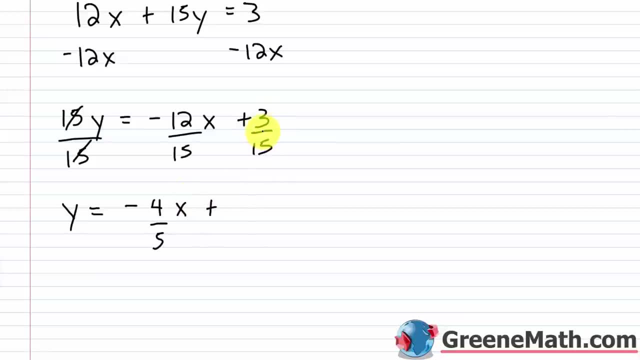 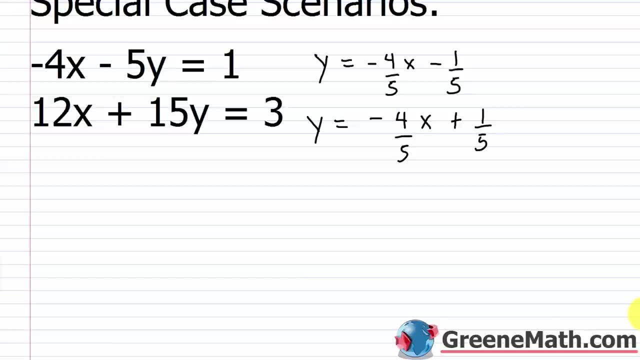 plus 3 15ths, Each is divisible by 3.. So I'll have 1 fifth. So it's really easy to make a mistake here and think that you have the exact same equation, but you don't. And what's different? 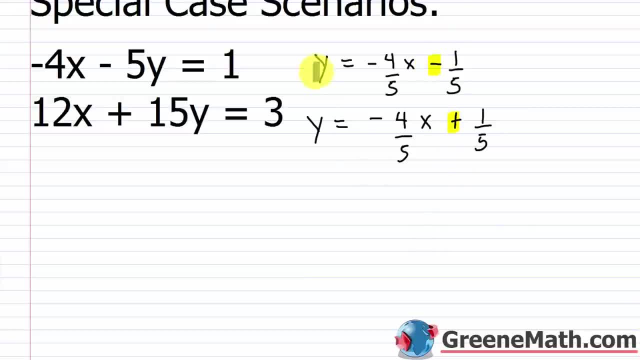 here is a minus and a plus. So you have y equals negative 4 fifths, x minus 1 fifth, So the y intercept occurs at 0 comma. For this one we have y equals negative 4 fifths, x plus. Okay, see how that's different. 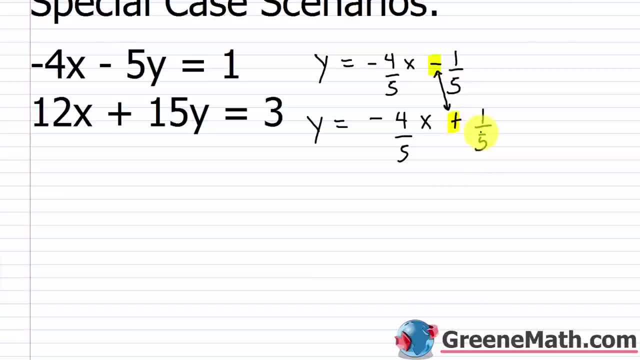 This is a minus, This is a plus 1 fifth. So the y intercept occurs here at 0 comma 1 fifth. So they're very similar but they're not the same equation, And so this is not a scenario where we have an infinite number of solutions. We don't have a solution at all. So these 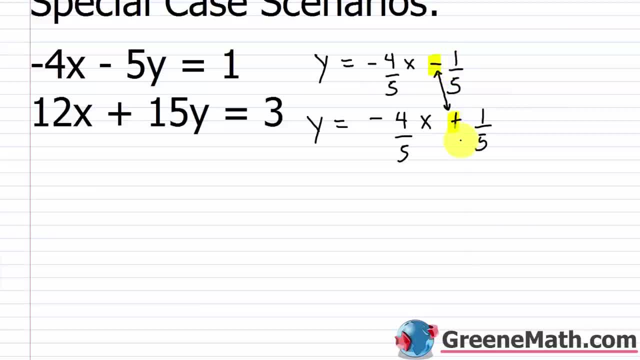 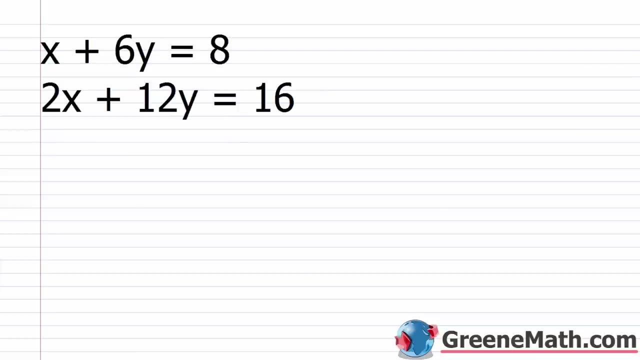 two equations will never cross on a coordinate plane. If you graph each one, they'll never touch each other. All right, so let's look at one. that's an infinite number of solutions, So some of you will get really good at this really quickly And you'll be able to spot that one of the equations is just a. 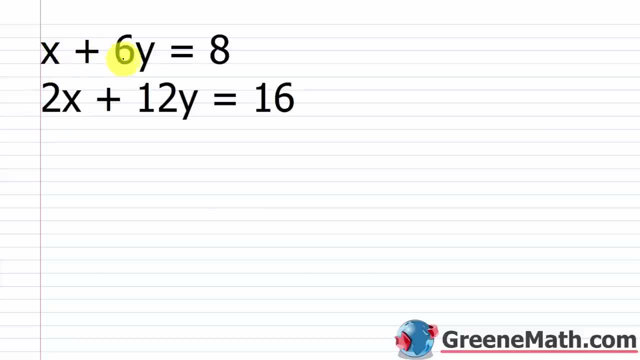 manipulated version of the other. So, in other words, if I look at, x plus 6y equals 8, and I multiply both sides of the equation by 2, I will get 2x plus 12y equals 16.. So it's the same thing. 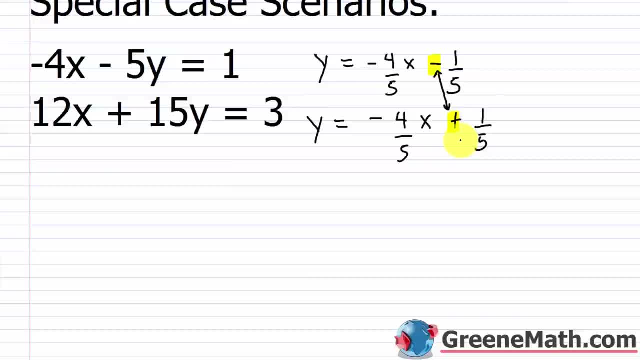 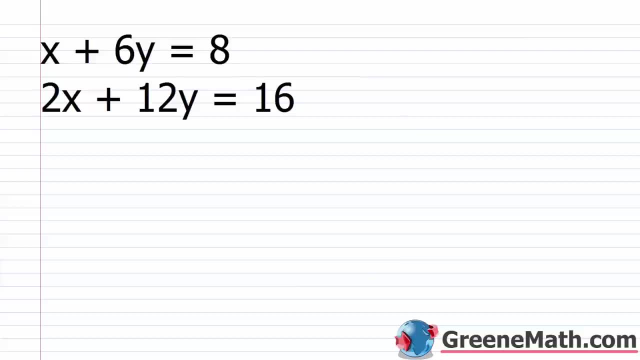 coordinate plane. If you graph each one, they'll never touch each other. You have two parallel lines. And so again, there's no solution. All right, so let's look at one that's an infinite number of solutions. So some of you will get really good at this really quickly, 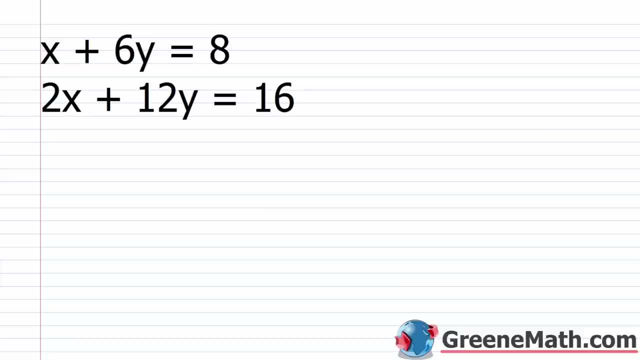 and you'll be able to spot that one of the equations is just a manipulated version of the other. So in other words, if I look at x plus 6y equals 8, and I multiply both sides of the equation by 2, I will get 2x plus 12y equals 16. So it's the same thing. I just took this equation and multiplied it by 2 to get to this equation. I'd have 2x plus 12y equals 16. 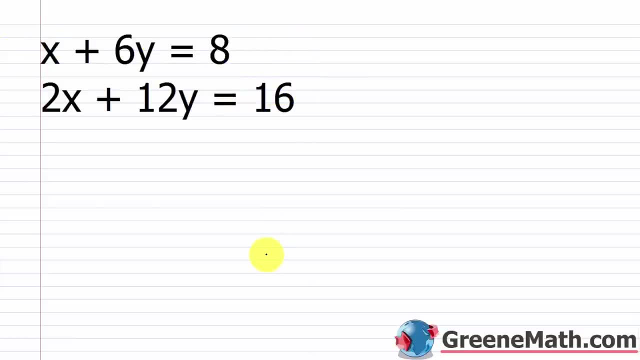 So now I'm going to look at this equation, and I'm going to multiply it with 16. So I'm going to take this sequence, and I'm going to multiply it with 16. So now I'm going to multiply knowing that in advance, I could just put that there's an infinite number of solutions because 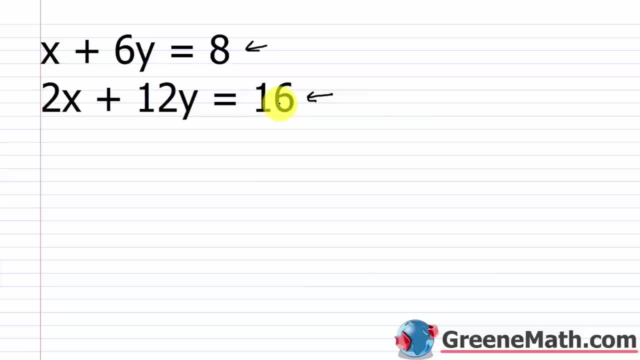 And a linear equation in two variables by itself has an infinite number of solutions. So in this particular case, again, the solution for the system would be an infinite number of 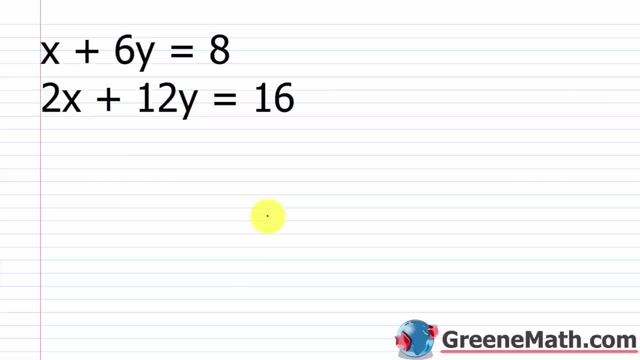 solutions. But let's go through and use substitution. I see that I have a coefficient of 1 for my variable x. So I'm going to go ahead and solve for that to start. So I'd have x. I'm going to go ahead and subtract 6y away from each side of the equation. So equals negative 6y plus 8. Again, all I did was subtract 6y from here and here. That's why I have a negative 6y on the right. So negative 6y plus 8. Now I'm going to plug this in for x in the other equation. So 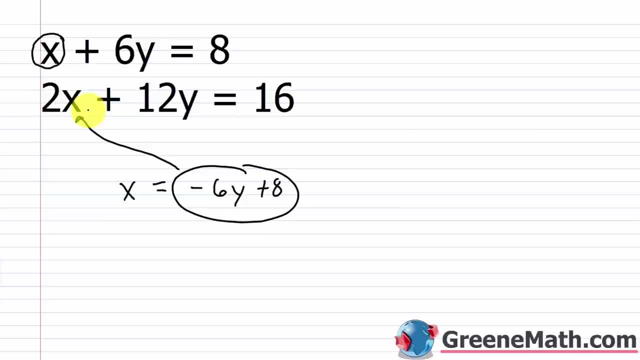 negative 6y plus 8. Again, that's a quantity. So I've got to use parentheses. So it's 2 times the quantity, negative 6y plus 8, then plus 12y equals 16. So 2 times negative 6y is 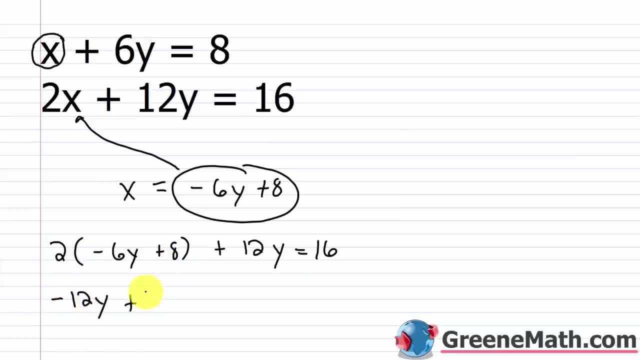 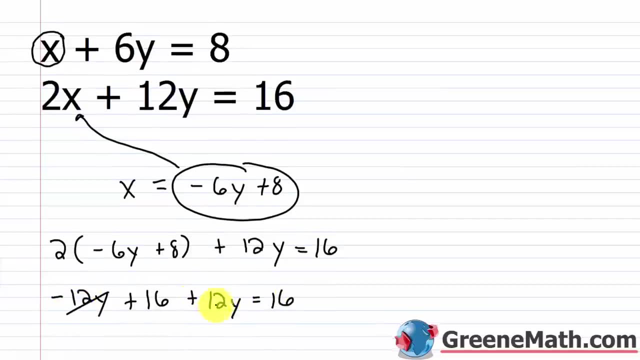 negative 12y. Plus 2 times 8, that's 16. Plus 12y equals 16. So negative 12y plus 12y, that's going to cancel. And I'm left with 16 equals 16. Or if I wanted to, I could subtract 16 away from each side and get 0 equals 0. It doesn't really matter. 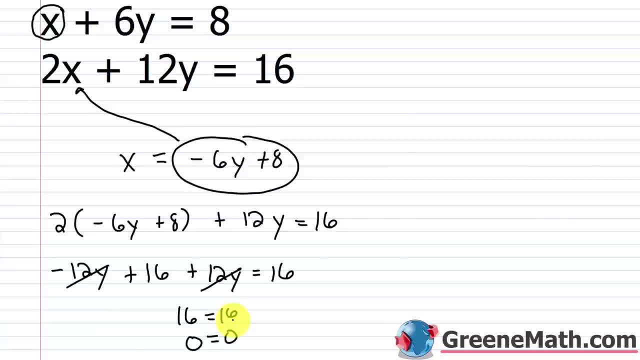 You get the same value on each side of the equation. You're left with a true statement. 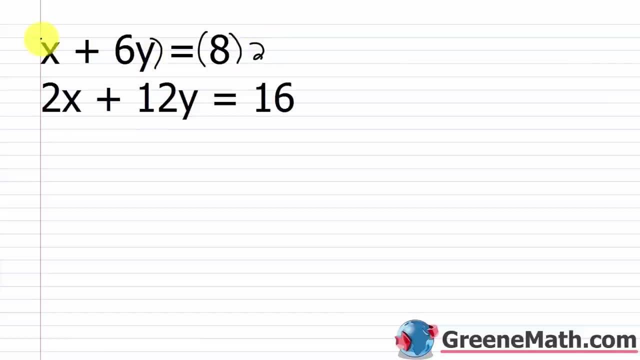 I just took this equation and multiplied it by 2. So I have: 2x plus 12y equals 16.. So, knowing that in advance, I could just put that there's an infinite number of solutions, because whatever works as a solution here is also going to work as a solution here. 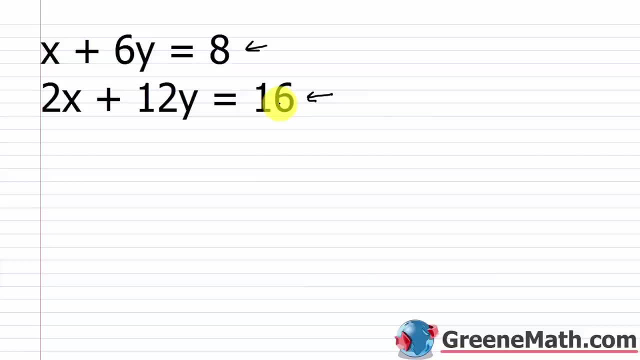 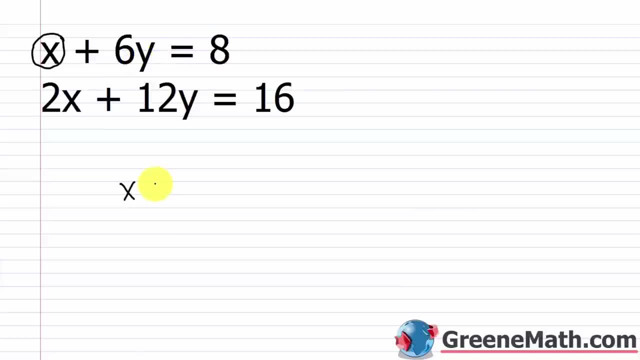 x. i'm going to go ahead and subtract 6y away from each side of the equation. so equals negative 6y plus 8 again. all i did was subtract 6y from here and here. that's why i have a negative 6y on the. 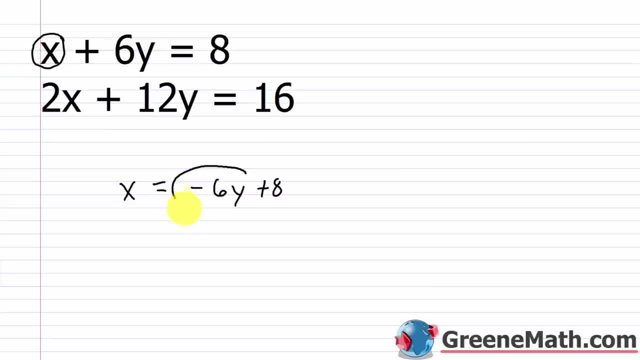 right. so negative 6y plus 8. now i'm going to plug this in for x in the other equation. so negative 6y plus 8. again that's a quantity, so i've got to use parentheses, so it's 2 times the quantity. 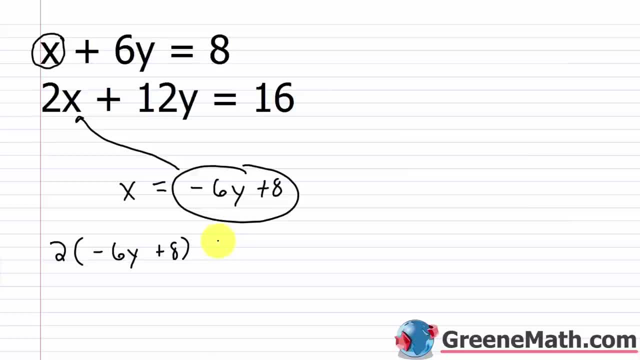 negative 6y plus 8, then plus 12y equals 16. so 2 times negative 6y is negative. 12y plus 2 times 8, that's 16 plus 12y equals 16. so negative 12y plus 12y, that's going to cancel. 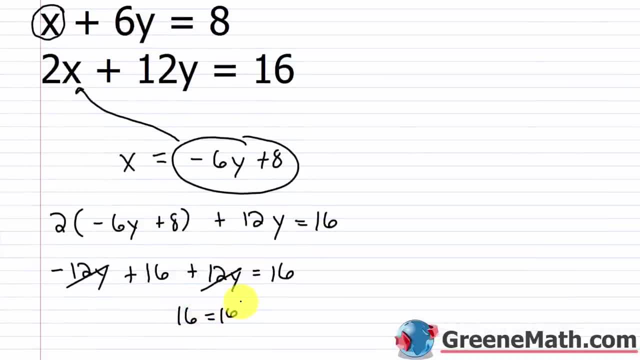 and i'm left with 16 equals 16, or, if i wanted to, i could subtract 16 away from each side and get 0 equals 0. doesn't really matter, you get the same value on each side of the equation. so i'm going to plug this in for x in the other equation, and i'm going to plug this in. 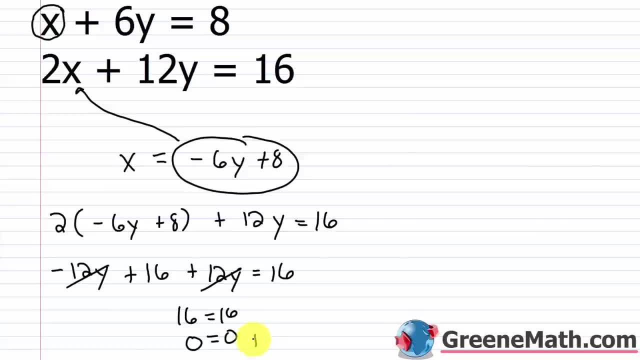 equation, You're left with a true statement. So yeah, this is true, Zero does equal zero or 16 does equal 16.. But it's not really what we're looking for. We're looking for a variable equal some number. So when the variables drop out and you're left with just a true statement, 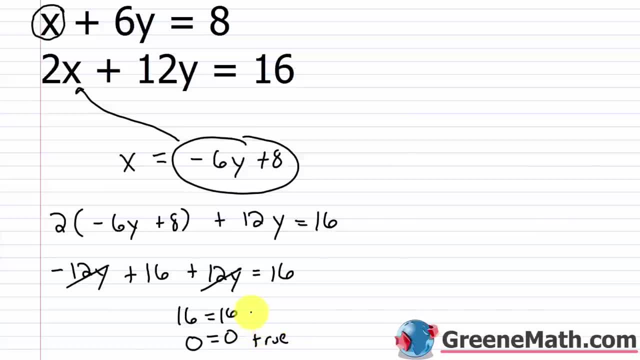 So yeah, this is true. 0 does equal 0. Or 16 does equal 16. But it's not really what we're looking for. We're looking for a variable equals some number. So when the variables drop out, and you're left with just a true statement, you know that you have a system that has an infinite number of solutions. The equations are what we call dependent. So there's an infinite number of solutions. 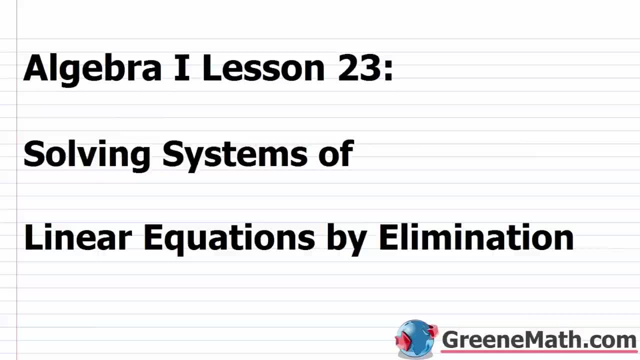 Hello, and welcome to Algebra 1, Lesson 23. In this video, we're going to learn about solving 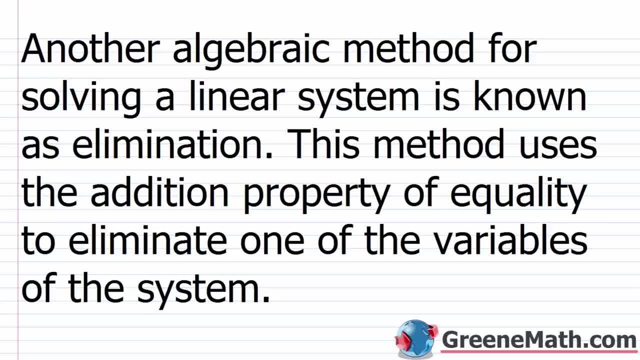 systems of linear equations by elimination. So in the previous two lessons, we learned about solving systems of linear equations by graphing, and then by substitution. So kind of the final method that we're going to talk about in Algebra 1 is known as elimination. So in this video, we're going to learn about solving systems of linear equations by elimination. So in the previous two lessons, we learned about solving systems of linear equations by graphing, and then by substitution. 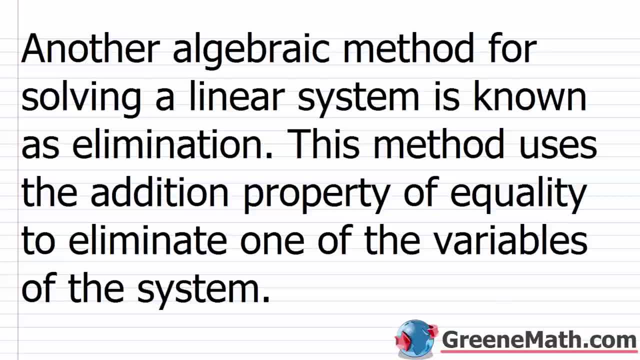 is known as elimination. So another algebraic method for solving a linear system is again known 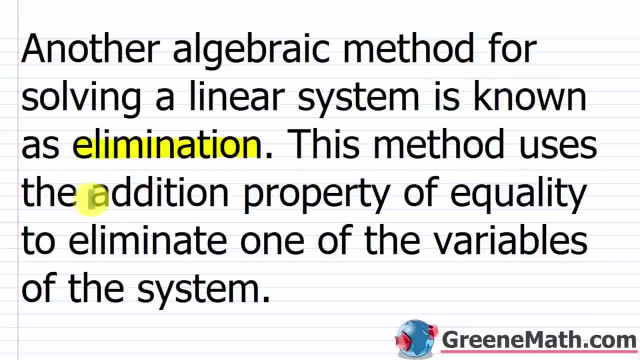 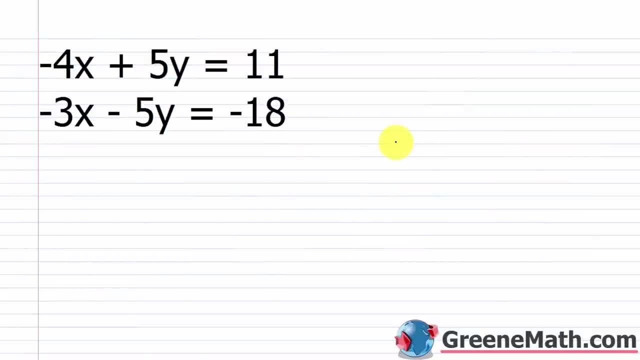 as elimination. So the method uses the addition property of equality to eliminate one of the variables of the system. So rather than start with kind of the textbook procedure, I want to 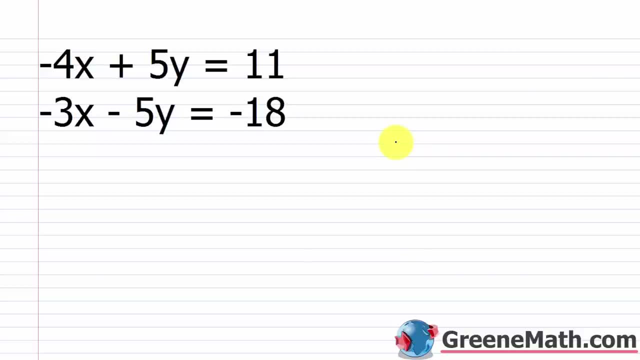 just look at two quick, nice, clean and easy examples. And I think we can learn the basics from this. 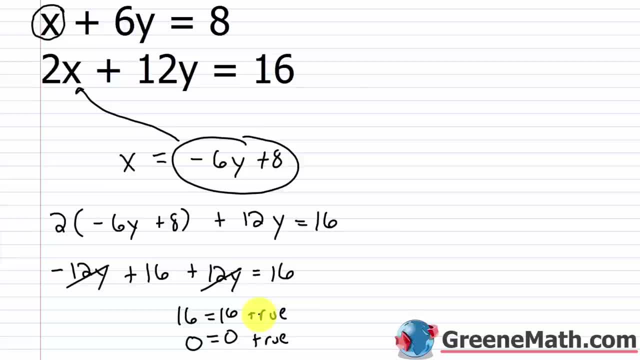 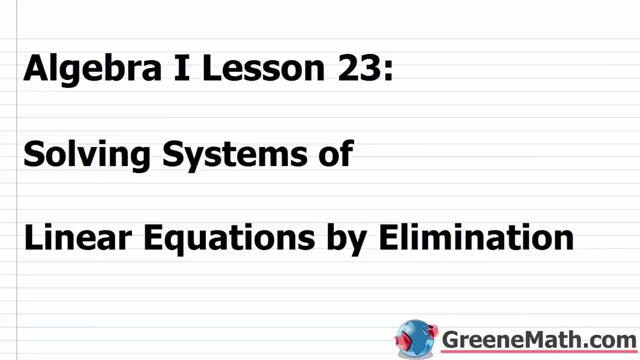 you know that you have a system that has an infinite number of solutions, right? The equations are what we call dependent, So there's an infinite number of solutions. Hello and welcome to Algebra 1,, Lesson 23.. In this video, we're going to learn about solving. 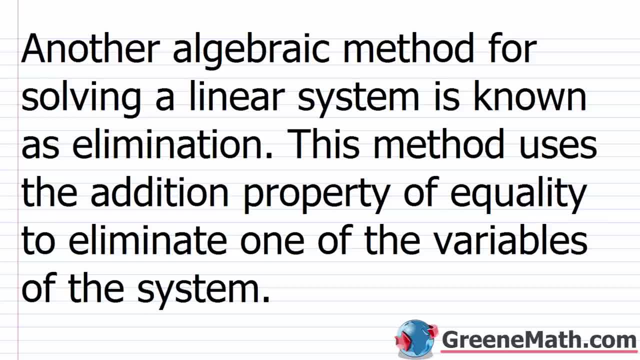 systems of linear equations by elimination. So in the previous two lessons we learned about solving systems of linear equations by graphing and then by substitution, So kind of the final method that we're going to talk about today is going to be the solution to the problem of. 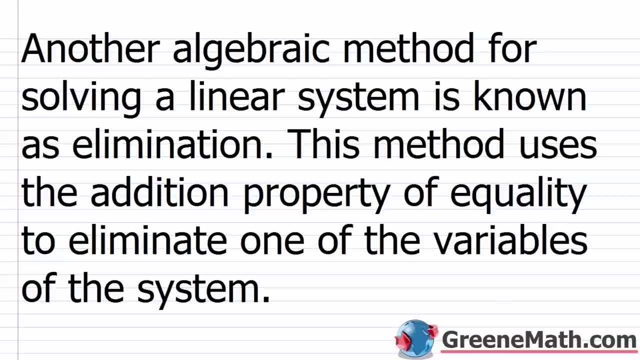 an Algebra 1 is known as elimination. So another algebraic method for solving a linear system is again known as elimination. So the method uses the addition property of equality to eliminate one of the variables of the system. So rather than start with kind of the textbook procedure, 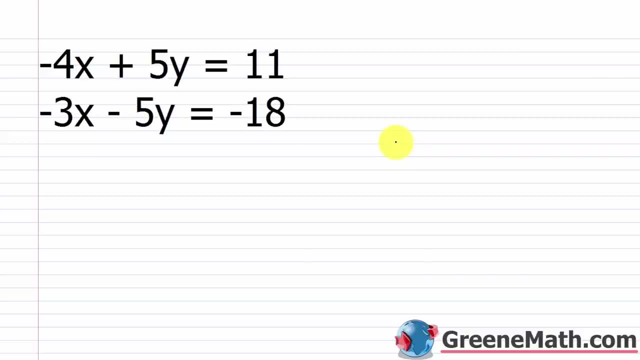 I want to just look at two quick, nice, clean and easy examples And I think we can learn the basics from this, Then go through kind of the textbook procedure and then, you know, move on to some harder problems. So I'm going to start out with this system that has negative: 4x plus 5y equals 11,. 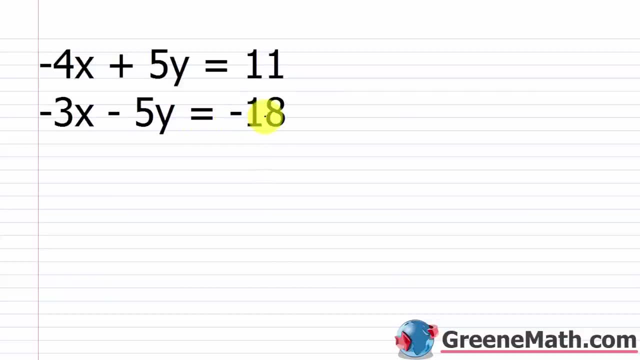 and negative 3x minus 5y equals negative 18.. So the first thing that I want to do when I'm using the elimination method is I want to take the left side of one of the equations and add it to the left side of the other equation. Now I'm going to label these for convenience. 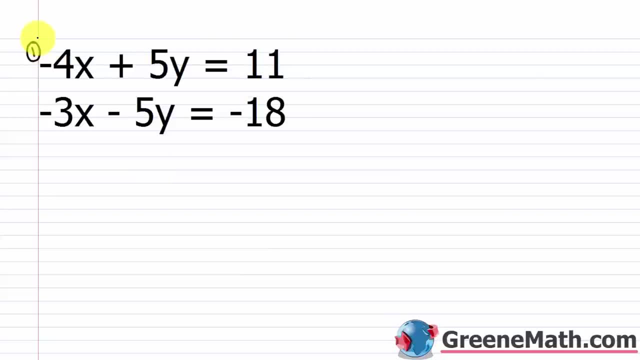 I'm going to label this top equation as equation one, just so I can refer to it, And this bottom equation as equation two, again just for reference sake. So I'm going to take the left side of equation one which is negative- 4x plus 5y- And I'm going to add to that the left side of equation. 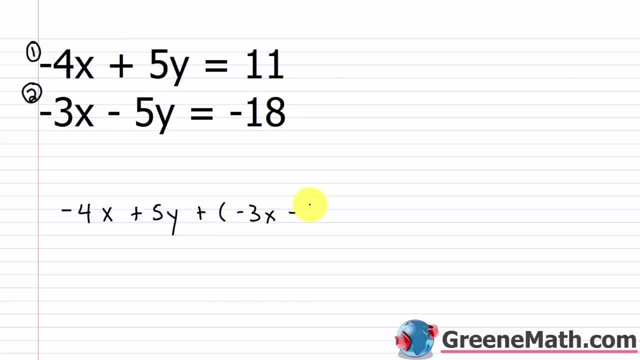 two, which is negative 3x minus 5y. Now I'm going to set this equal to the sum of the two right sides. So the right side of equation one is 11.. And then the right side of equation two is negative 18.. 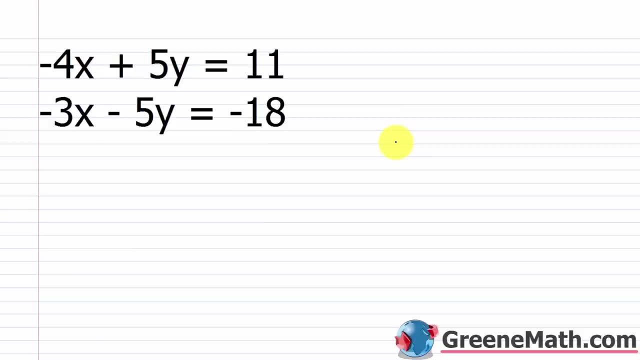 So we're going to go through kind of the textbook procedure and then, you know, move on to some harder problems. So I'm going to start out with this system that has negative 4x plus 5y equals 11 and negative 3x minus 5y equals negative 18. So the first thing that I want to do when I'm using the elimination method is I want to take the left side of one of the equations and add it to the left side of the other equation. Now, I'm going to label these for convenience. I'm going to label this top equation as equation is equal to 1. And I'm going to label these as equal to 1. So I'm going to label these as equal to 1. And I'm going to label these as equal to 1. And I'm going to label these as equal to as equation one, just so I can refer to it. And this bottom equation is equation two, again, just for reference sake. So I'm going to take the left side of equation one, which is negative four x plus five y. And I'm going to add to that the left side of equation two, which is negative three x minus five y. I'm going to set this equal to the sum of the two right sides. So the right side of equation one is 11. And then the right side of equation two is negative 18. So what's going to happen here is that one of the variables is going to drop out. And specifically, the reason for that is because the coefficients are opposites. Okay, so let's do our addition here. Negative four x plus negative three x is negative seven x. And then five y plus negative five y is zero, right? 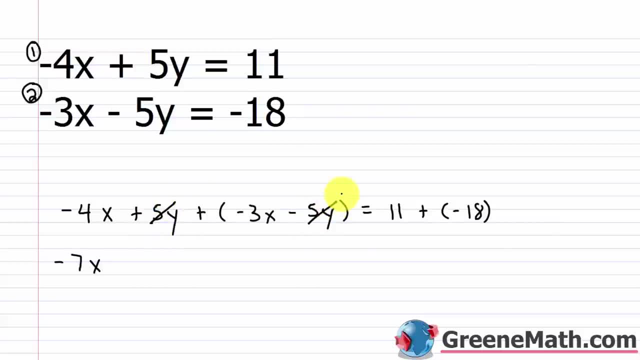 So this variable here, y has been eliminated. So we have negative seven x is equal to we have 11 plus negative 18. That's negative seven. So just that quick, we have a linear equation one variable. 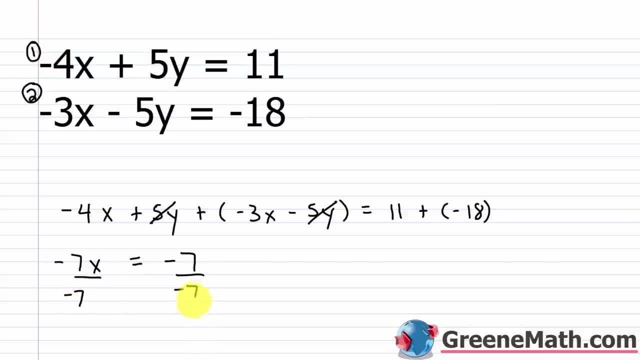 And we can solve this very quickly for x, divide both sides by negative seven, the coefficient of x, that will cancel, and I will have x is equal to one. 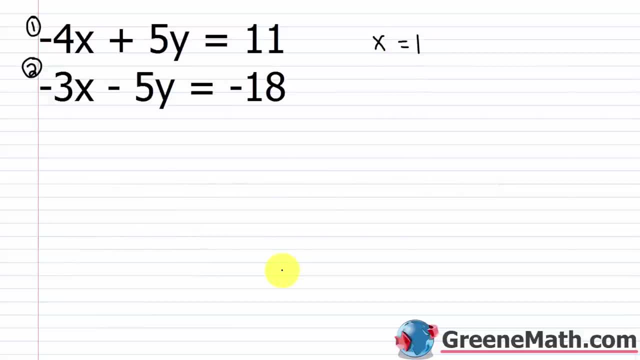 All right, so just from using some common sense, now, you can kind of think about what we would do to get y, if one is the value for x, for my solution for the system, that means I can plug a one in for x in either original equation. And I can solve for y, right, I'd have a linear equation with just y in it. Very easy to solve for that. So let's just plug it into the first equation, we'd have negative 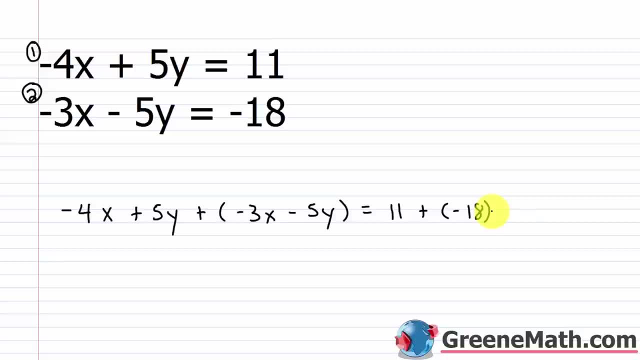 So what's going to happen here is that one of the variables is going to drop out, And specifically the reason for that is because the coefficients are opposites. Okay, So let's do our addition here: Negative 4x plus negative 3x is negative 7x, And then 5y plus negative 5y is zero. 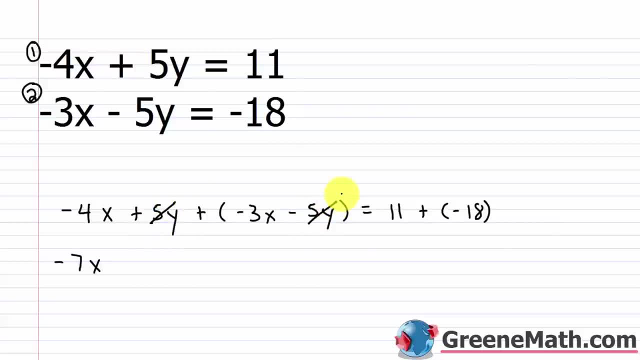 Right. So this variable here, y, has been eliminated. So we have negative 7x is equal to, we have 11 plus negative 18.. That's negative 7.. So just that quick. we have a linear equation, one variable And we can solve this very quickly: for x, Divide both sides by negative 7,. 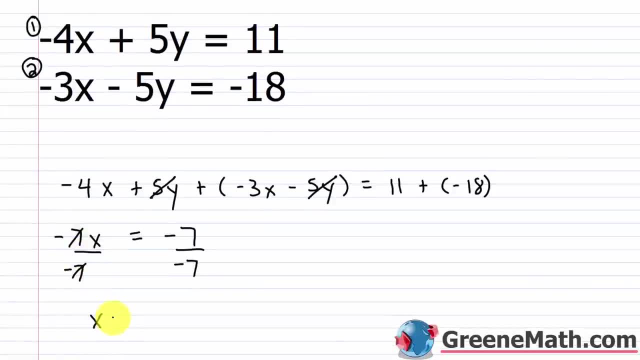 the coefficient of x. That will cancel And I will have x is equal to 1.. All right, So just from using some common sense now you can kind of think about what would we do to get y If 1 is the value for x? for my solution, for the system, that means I can plug a 1 in for 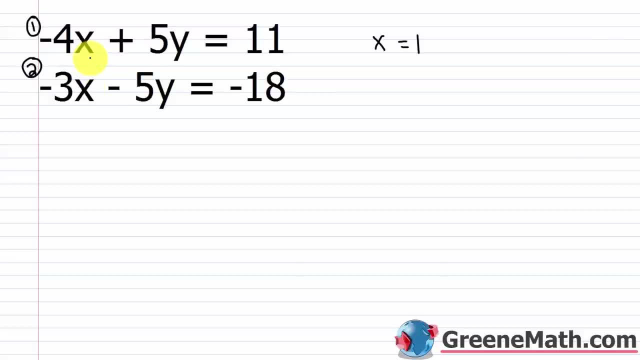 x in either original equation And I can solve for y Right. I'd have a linear equation with just y in it. Very easy to solve for that. So let's just plug it into the first equation. We'd have negative 4 times 1, just plugging in a 1 for x plus 5y equals 11.. 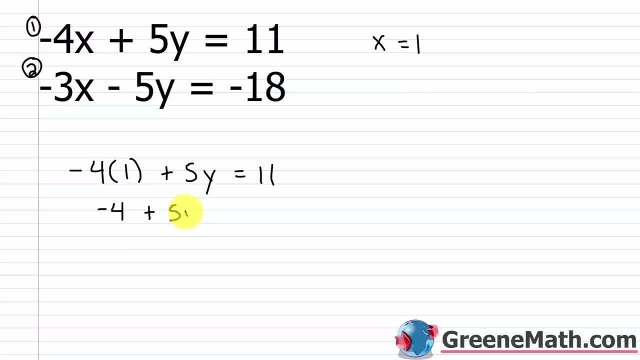 Negative 4 times 1 is negative 4, plus 5y equals 11.. Add 4 to both sides of the equation. That's going to cancel. I'll have: 5y is equal to 11 plus 4 is 15.. 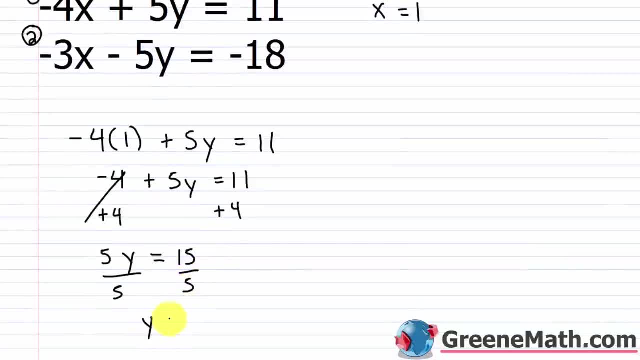 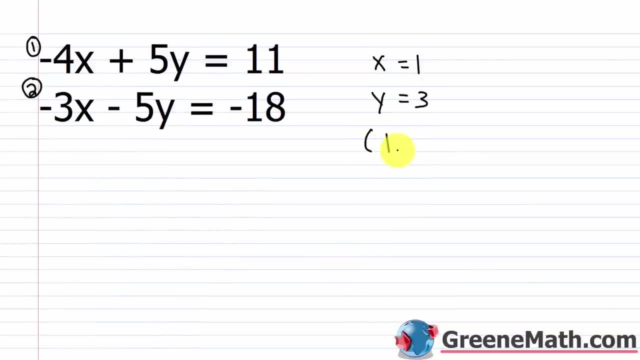 Divide both sides of the equation by 5. And you're going to get that y is equal to 3.. So this represents the ordered pair 1, 3.. And before I move on and kind of explain why I did what I did, I'm going to go ahead and do a little bit of a test. 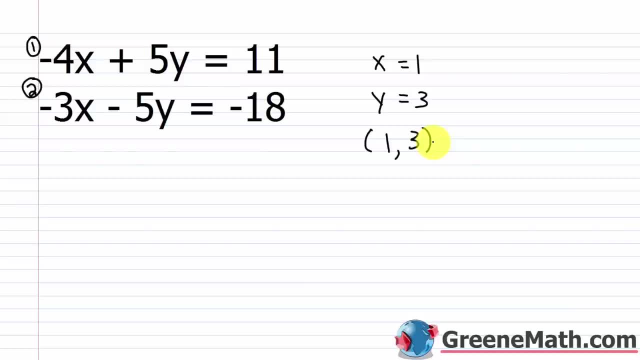 And why it's legal. I want to go in and check 1,, 3, that ordered pair in each equation of the system. So let's start out with equation 1.. We'd have negative 4 times 1 plus 5 times 3 is equal to 11.. Negative 4 times 1 is negative 4, plus 5 times 3 is 15,. 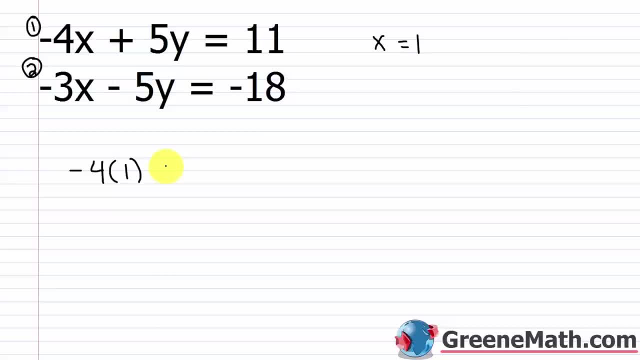 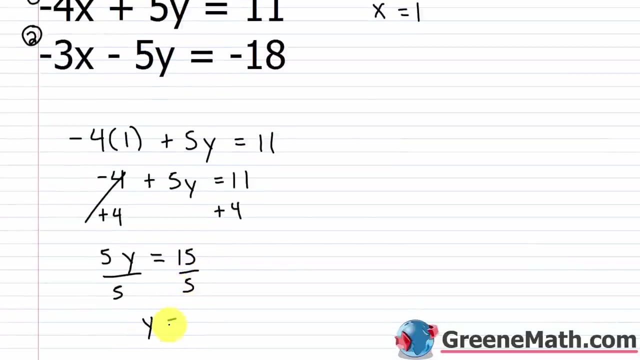 four times one, just plugging in a one for x, plus five y equals 11. Negative four x is negative seven, four times one is negative four, plus five y equals 11. Add four to both sides of the equation, that's going to cancel, I'll have five y is equal to 11 plus four is 15. Divide both sides of the equation by five, and you're going to get that y is equal to three. So this represents the ordered 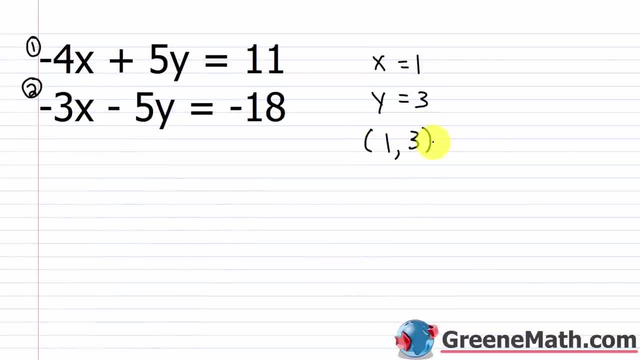 pair, one comma three. And before I move on and kind of explain why I did what I did, and why it's legal, I want to go in and check one comma three, that ordered pair, in each equation of the 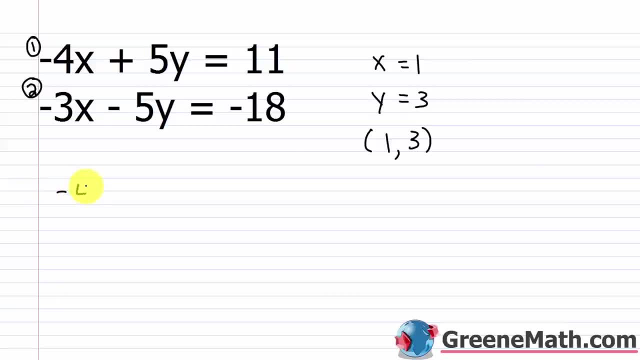 system. So let's start out with equation one, we'd have negative four times one, plus five times three, is equal to 11. Negative four times one is negative four, plus five times three is 15, equals 11. Negative four plus 15 is 11, so you get 11 equals 11. So yes, does work as a solution for this first one. All right, for the second one, I have a negative three x, so that's negative three times one, minus five y, so that's minus five times three, this equals negative 18. So negative three times one is negative three. And then we have minus five times three is 15. And this equals negative 18. And it does negative three minus 15 is negative 18. So you get negative 18 equals negative 18. So it works out here as well. So now that we've verified this equation, we're going to go ahead and do the next one. So we're going to go ahead 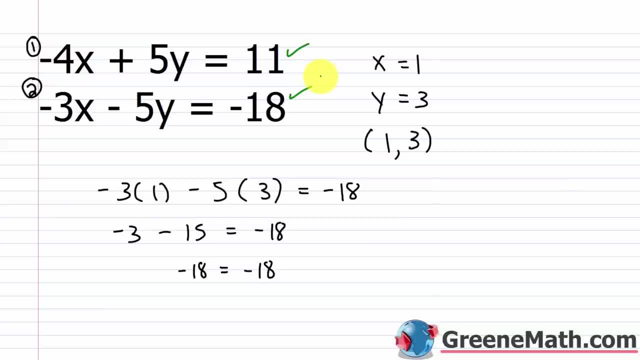 that one comma three, that ordered pair is a solution for the system. Let's talk about what we did to get it and why this method is mathematically legal. So the very first thing I want to call your attention to is that these two equations are set up in standard form, right? It's ax plus by equals c. And I know some of you are going to scream and say, well, that's not standard form. This isn't greater than or equal to zero. Okay, I'm talking about standard form where we don't have any real numbers. Okay, just for this section, I want you to just think about it as a, b, 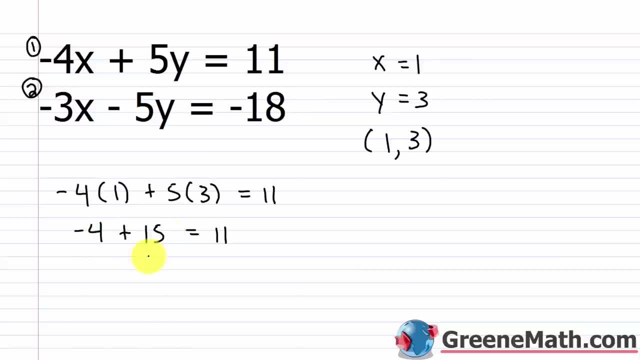 equals 11.. Negative 4 plus 15 is 11.. So you get 11 equals 11.. So, yes, it does work as a solution for this first one, All right. for the second one, I have negative 3x, So that's negative 3 times 1,. 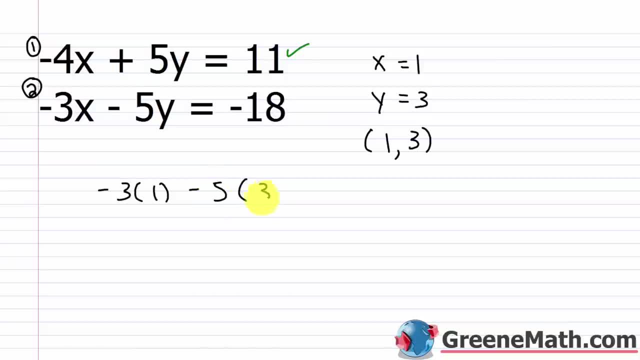 minus 5y, So that's minus 5 times 3. And this equals negative 18.. So negative 3 times 1 is negative 3.. And then we have: minus 5 times 3 is 15. And this equals negative 18. And it does. 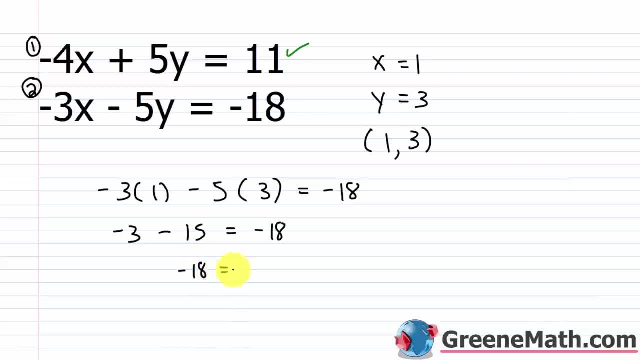 Negative 3 minus 15 is negative 18.. So you get negative 18 equals negative 18.. So it works out here as well. So now that we've done that, let's go ahead and do the next one. So, let's do the next one. 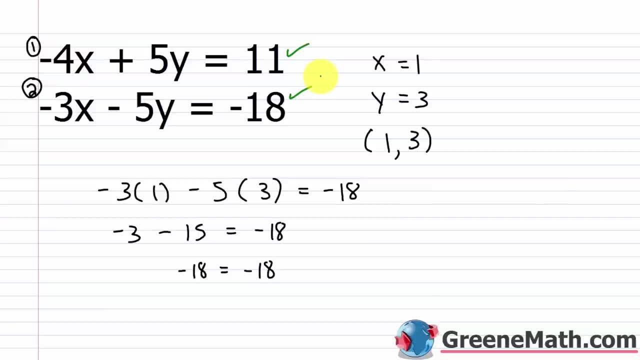 So let's do the next one. So, now that we've verified that 1 comma 3, that ordered pair, is a solution for the system, Let's talk about what we did to get it and why this method is mathematically legal. 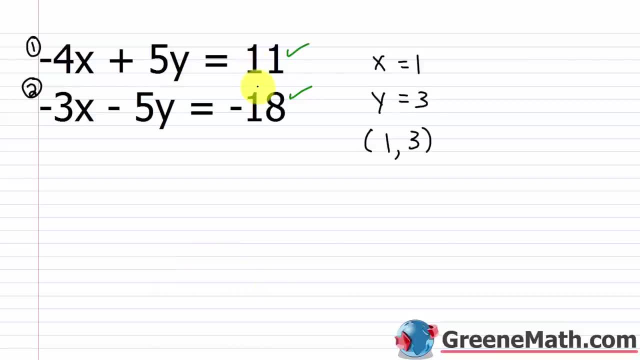 So the very first thing I want to call your attention to is that these two equations are set up in standard form. right, It's ax plus by equals c, And I know some of you are going to scream and say, well, that's not standard form. This isn't greater than or. 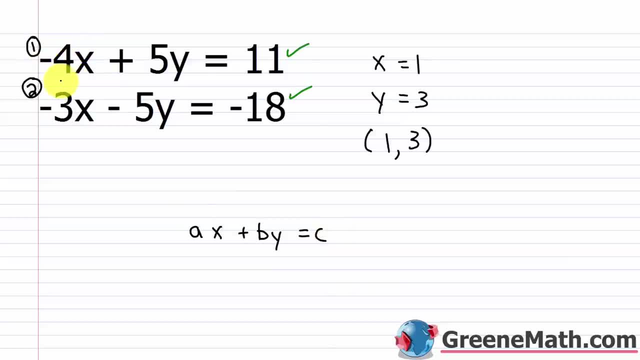 equal to zero. Okay, I'm talking about standard form, where we just think about a, b and c as real numbers. Okay, Just for this section, I want you to just think about it as a, b and c just being real numbers, And a and b just can't both be zero. Okay, That's your. 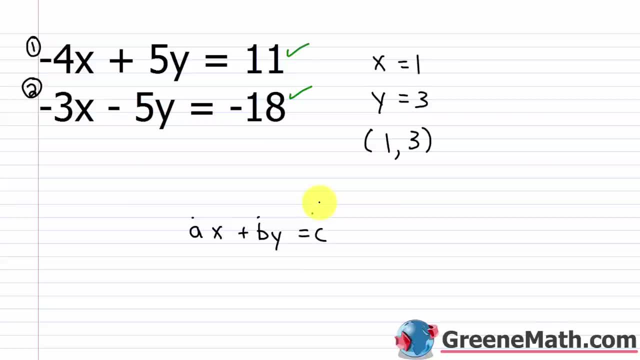 only restriction. So once we have them both set up in this format, when you put the two on top of each other, it's going to be very easy to see right away if one of the variables would be eliminated through addition. And how do you tell that? Well, you look at the coefficients. 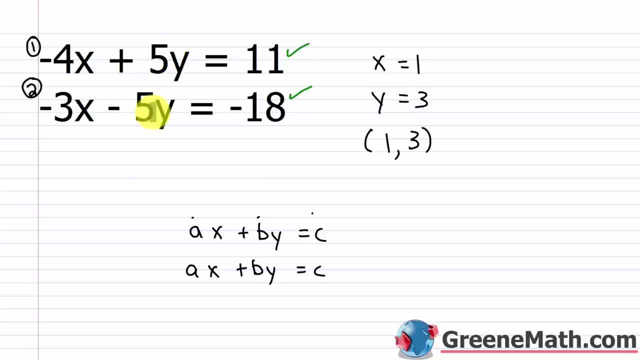 If one pair have opposite coefficients. So in other words, this y variable here has a coefficient of five. This y variable here has a coefficient of negative five. So obviously if I add five and negative five that's going to be zero. So I'd have zero y or just zero If I have negative three. 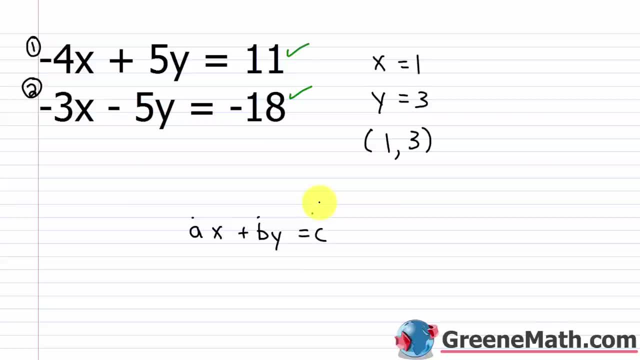 and c just being real numbers. And a and b just can't both be zero. Okay, that's your only restriction. So once we have them both set up in this format, when you put the two on top of each other, it's going to be very easy to see right away if one of the variables would be eliminated through addition. And how do you tell that? Well, you look at the coefficients. If one pair have opposite coefficients, so in other words, this y variable here has a coefficient of five. This y variable here has a coefficient of negative five. So obviously, if I add five and negative five, that's going to be zero. So I'd have zero y or just zero. If I have negative three and positive three, that's zero. If I have negative 212 and positive 212, that's going to be zero. We know that if we add a number and it's opposite, it's zero. So if I see one pair of variable terms with opposite coefficients, I know that this is going to be a very quick and easy method to get a solution for the system. So let me erase this real quick. And let's talk about why this is legal now. Because this is probably the thing that trips students up the most. They say, well, how are you able to add this side to that side? And that doesn't make any sense. Why are we able to do that? Well, mathematically, if I took the first equation and said negative five, I'd have zero. So if I took the first equation and said negative five, 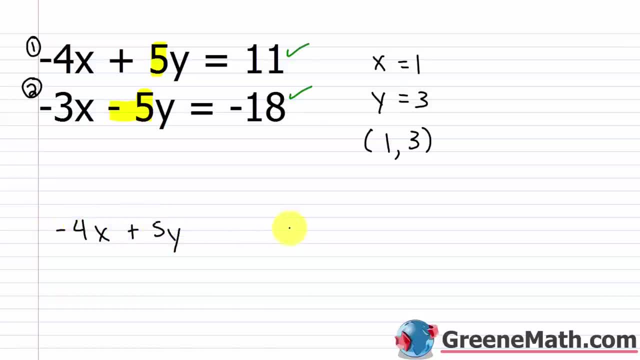 four x plus five y equals 11. You recall that the addition property of equality tells us that we can add the same quantity or the same amount to both sides of an equation, and we won't change the solution. So in other words, I could add three to both sides of this equation. And anything that was a solution before is now still a solution. So kind of expanding on that, 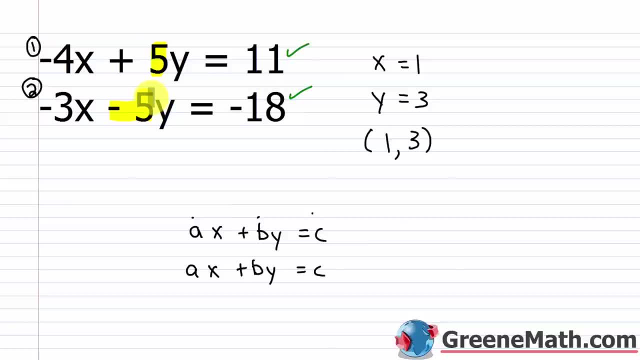 and positive three, that's zero. If I have negative 212 and positive 212, that's going to be zero. We know that if we add a number and it's opposite, it's zero. So if I see one pair of variable terms with opposite coefficients, I know that this is. 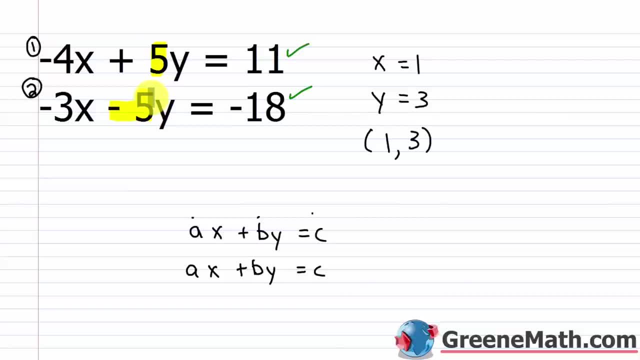 going to be a very quick and easy method to get a solution for the system. So let me erase this real quick And let's talk about why this is legal now, because this is probably the thing that trips students up the most. They say, well, how are you able to add this side to that side? 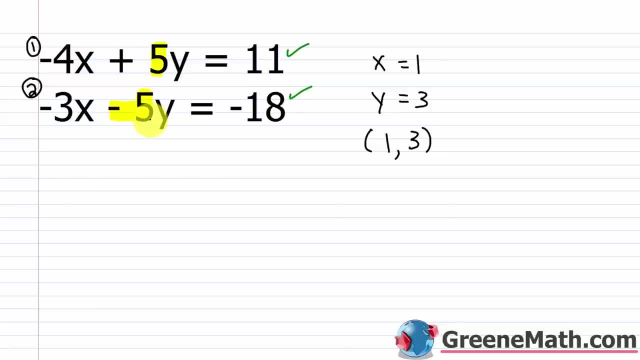 And that that doesn't make any sense. Why are we able to do that? Well, mathematically, if I took the first equation and said negative, four x plus five y equals 11, you recall that the addition property of equality tells us that we can add the same quantity or the same amount to both sides of. 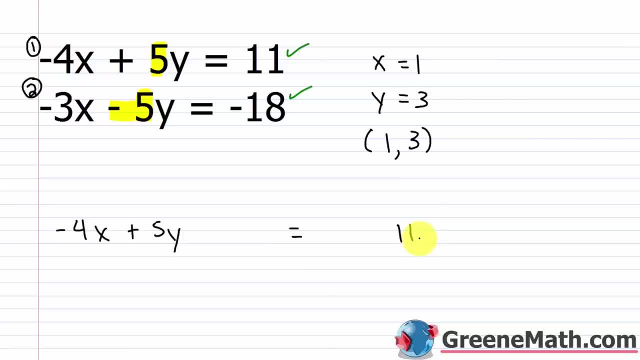 an equation and we won't change the solution. So in other words, I could add three to both sides of this equation And anything that was a solution before is now still a solution. So, expanding on that, if I think about equation two for a moment and I look at this equal sign. 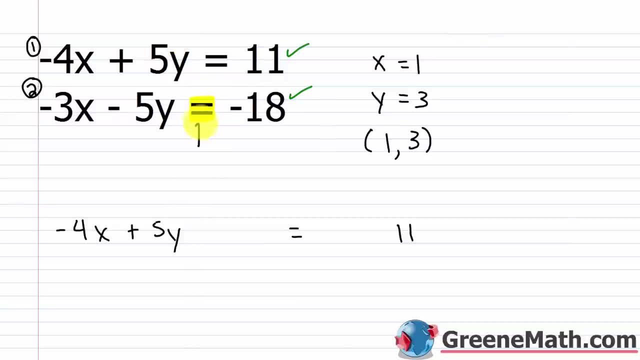 let's think about this for a second. This equal sign means the same as, the same as. So that means that we are saying negative three x minus five y is the same as negative 18. So they represent the same quantity. So what that means is that I can add this: 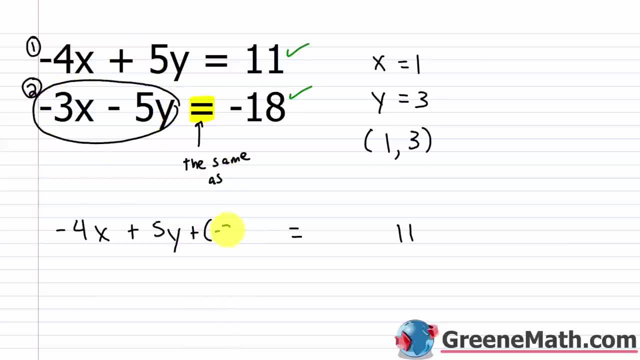 to this side of the equation. So plus negative three x. let me kind of scooch this down a little bit- minus five y and add this to the other side of the equation And I've added the same quantity. This is equal to this, So I can add them to both sides of the equation. legally It's the same thing. 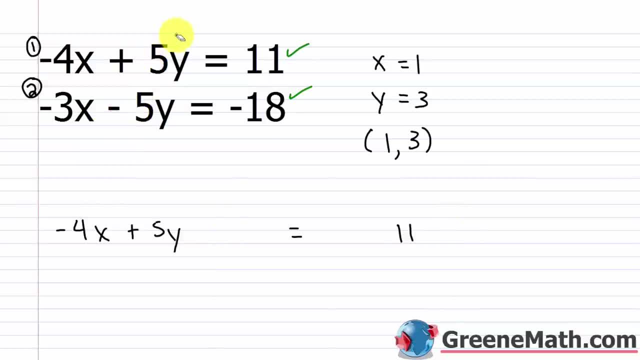 if I think about equation two for a moment, and I look at this equal sign, let's think about this for a second. This equal sign means the same as, the same as. So that means that we are saying negative three x minus five y is the same as negative 18. So they represent the same quantity. So what that means is that I can add this to this side of the equation. So I can add this to the other side of the equation, and I've added the same quantity. This is equal to 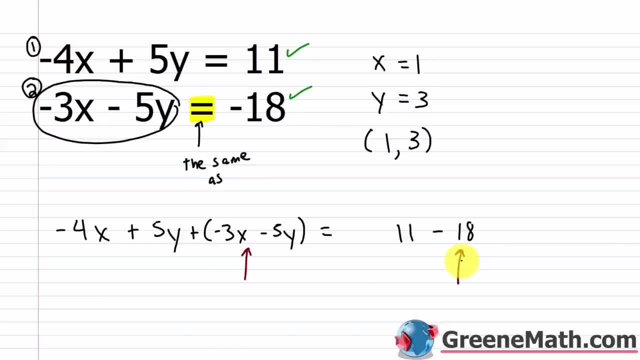 this. So I can add them to both sides of the equation legally. It's the same thing as when I added three to both sides of the equation. It represents the same amount or the same quantity. 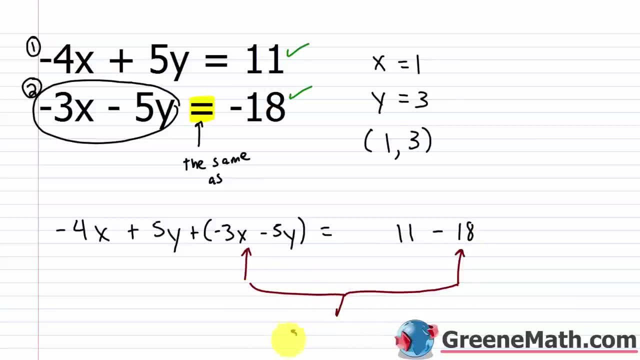 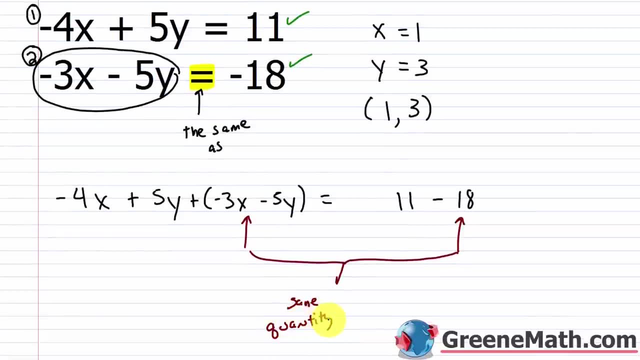 So let me kind of draw that like that and put same, quantity. Okay. So that's why we're legally able to do that. So using this strategy, if we have one pair of variable terms with opposite coefficients, it's going to drop out, and it's going to leave me with a linear equation of one variable that I can then solve. In this case, we solved and we found that x was equal to one. Then I can plug that back in for x in any of the original equations, and I can figure out what the other unknown is. All right, 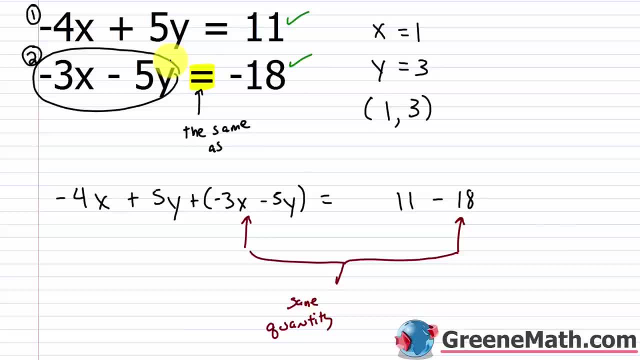 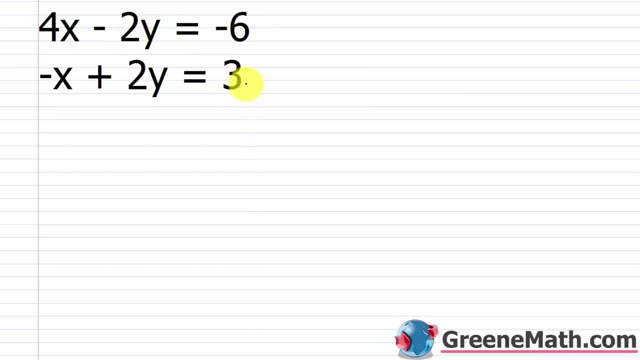 let's take a look at another one. And again, we're going to look at another easy one. And we have 4x minus 2y equals negative 6. We have negative x plus 2y equals 3. So again, you see I wrote it in the format of ax plus by equals c, ax plus by equals c. Okay, so it's already set up for you like that. Now, right away, if you kind of look at things, I have a coefficient of 4 here and a coefficient of negative 1 here. So those aren't opposites, 4, negative 1, negative 2, negative 1, are not opposites. I have a coefficient of negative 2 here and a coefficient of positive 2 here. Those are opposites. So negative 2 plus 2 is 0. So I know when I do my first step, I add the two left sides together, this variable is going to be eliminated. Now, kind of a quicker way to do 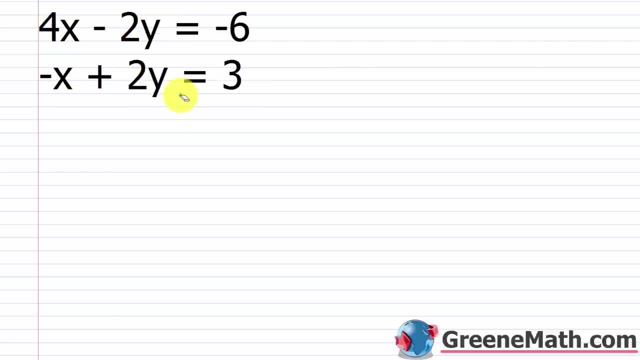 this, and a lot of students prefer to use this method, you can add vertically. Okay, so you can 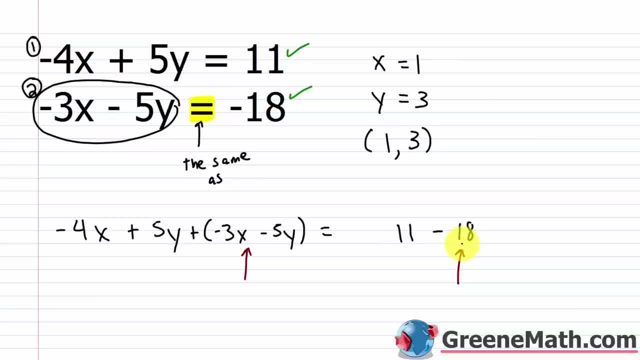 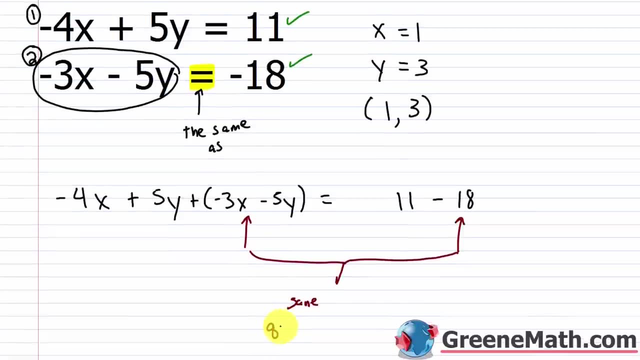 as when I added three to both sides of the equation It represents the same amount or the same quantity. So let me kind of draw that like that And I can add this to the other side of the equation. So that's why we're legally able to do that. So, using this strategy, if we have one pair, 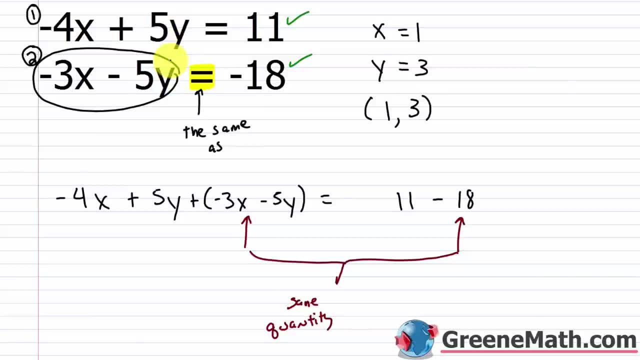 of variable terms with opposite coefficients, it's going to drop out and it's going to leave me with a linear equation of one variable that I can then solve. In this case, we solved and we found that x was equal to one. Then I can plug that back in for x in any of the original equations. 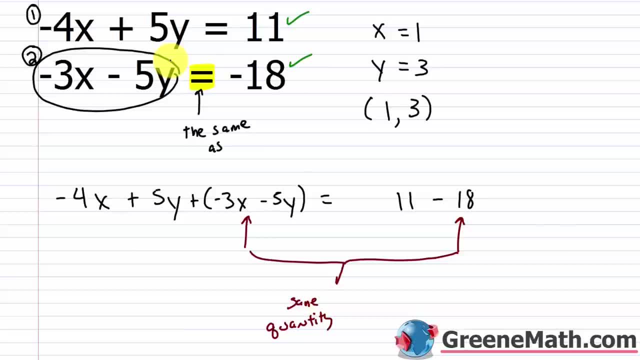 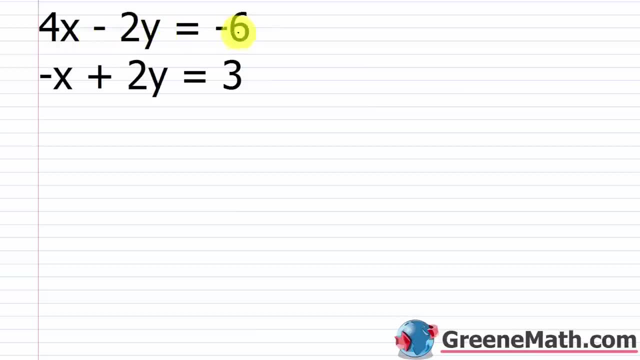 And I can figure out what the other unknown is. All right, let's take a look at another one. and again we're going to look at another easy one. and we have 4x minus 2y equals negative 6. we have negative x plus 2y equals 3.. So, again, you. 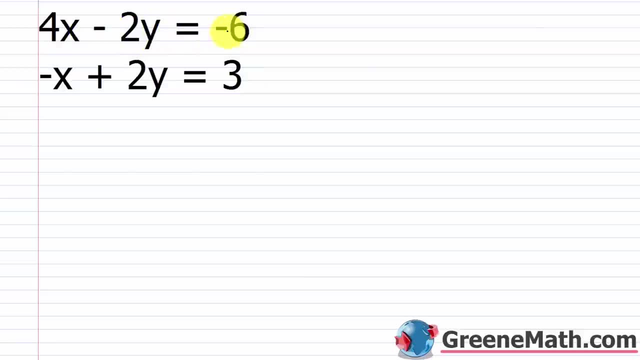 see, I wrote it in the format of ax plus by equals c, ax plus by equals c. Okay, so it's already set up for you like that. Now, right away, if you kind of look at things, I have a coefficient of 4 here and a coefficient of negative 1 here. So those aren't opposites. 4 and negative 1 are not. 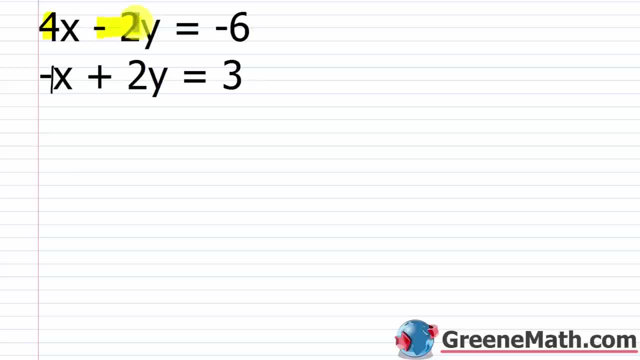 opposites. I have a coefficient of negative 2 here and a coefficient of positive 2 here. Those are opposites. So negative 2 plus 2 is 0. So I know, when I do my first step, I add the two left sides together. this variable is going to be eliminated. Now kind of a quicker way to do this. 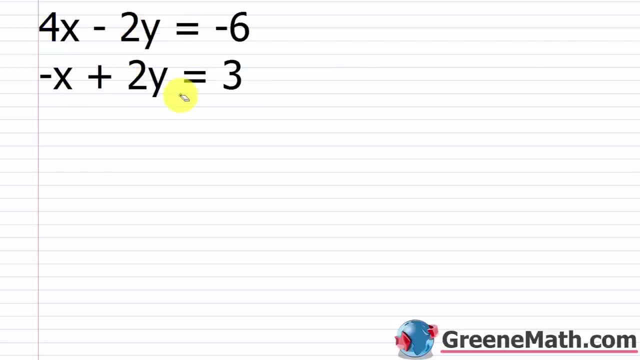 and a lot of students prefer to use this method. You can add variable Vertically, Okay, so you can kind of just add it the way it's set up. You can put a plus sign out here if you want. You don't need to, I never do. I just add going down. So 4x plus negative x. 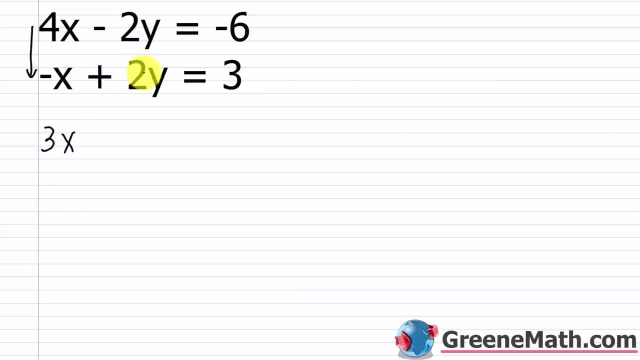 is 3x Negative. 2y plus 2y is 0y, So that's eliminated and this is equal to negative 6 plus 3 is negative 3.. So now I have a linear equation of one variable and I can divide both. 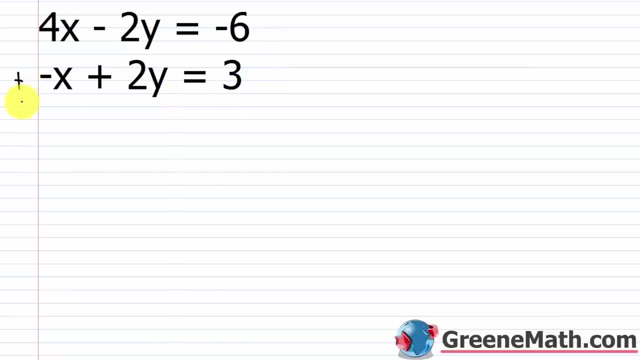 kind of just add it the way it's set up. You can put a plus on it, you can put a minus on it, you can put a minus on it. I know I've talked about this a lot in your classes, but I'm gonna give you the given sign out here. If you want, you don't need to. I never do. I just add going down. So 4x plus negative x is 3x, negative 2y plus 2y is 0y, so that's eliminated. And this is equal to negative 6 plus 3 is negative 3. So now I have a linear equation of one variable, and I can divide both sides by 3, the coefficient of x, and get that x is equal to negative 1. find that x equals negative 1, I can plug a negative 1 in for x in either of the original equations, solve for y. So let's go ahead and plug into this second equation. Looks like it's easier to work with. We have negative, and then I'm plugging in a negative 1. So minus a negative 1 would be plus 1, then plus 2y equals 3. I'm going to subtract 1 away from each side. That's gone. I'll have 2y is equal to 2. Divide both sides of the equation by 2, and I'm going to get that y is equal to 1. So this is the ordered pair negative 1 comma 1. Again, let's check to make sure we got the right answer. So I have 4x minus 2y equals negative 6. So I'd have 4 times negative 1 minus 2 times positive 1 equals negative 6. 4 times negative 1 is negative 4. So negative 4 minus 2 times 1. 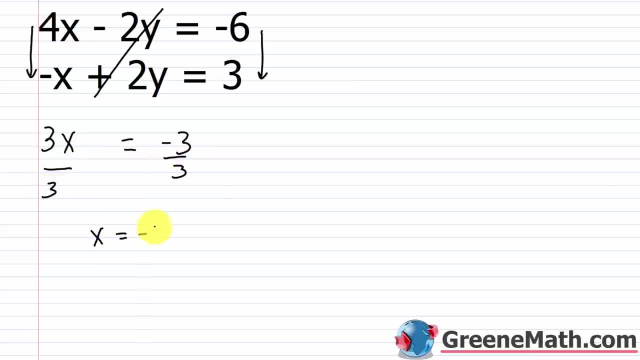 sides by 3 the coefficient of x And get that x is equal to negative 1.. So once I find that x equals negative 1, I can plug a negative 1 in for x. in either of the original equations Solve for y, So let's go ahead and plug into this second equation. Looks like it's. 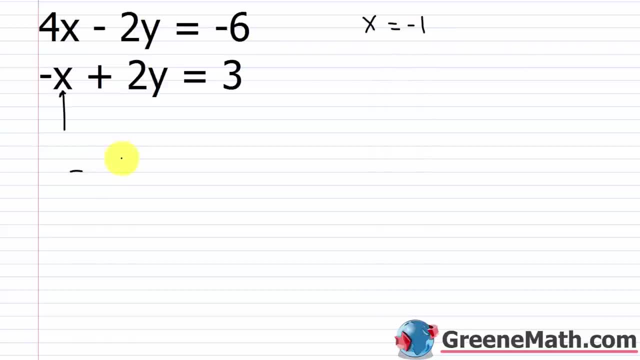 easier to work with. We have negative, and then I'm plugging in a negative 1.. So minus a negative 1 would be plus 1. Then plus 2y equals 3.. I'm going to subtract 1 away from each side. 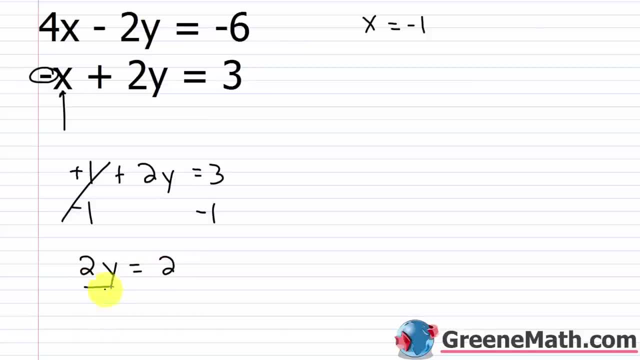 That's going to be negative 1.. So I'm going to plug in a negative 1.. So I'm going to plug in a negative 1.. I'll have: 2y is equal to 2.. Divide both sides of the equation by 2.. And I'm going to get that y is. 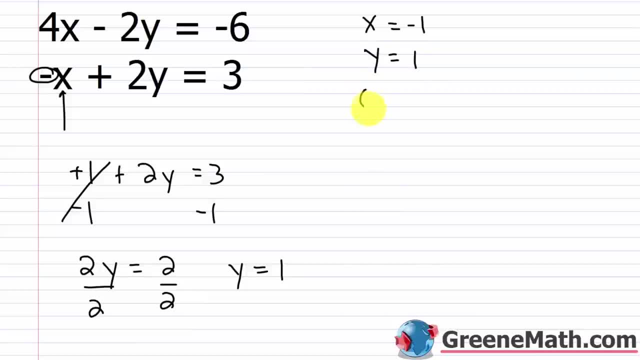 equal to 1.. So this is the ordered pair: negative 1 comma 1.. Again, let's check to make sure we got the right answer. So I have 4x minus 2y equals negative 6. So I'd have 4 times negative 1 minus. 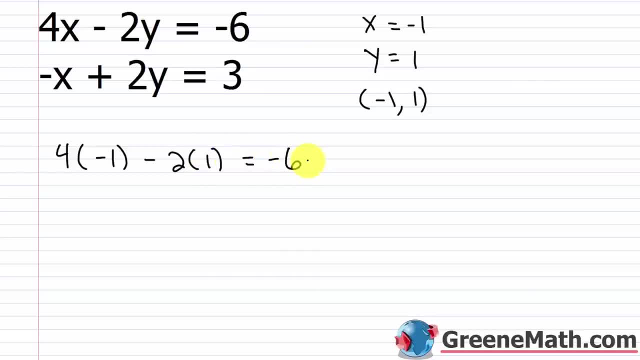 2 times positive, 1 equals negative 6. 4 times negative, 1 is negative 4. So negative 4 minus 2 times 1 is negative, 6. So you get negative 6 equals negative, 6. So it checks out in the first one. Let's take 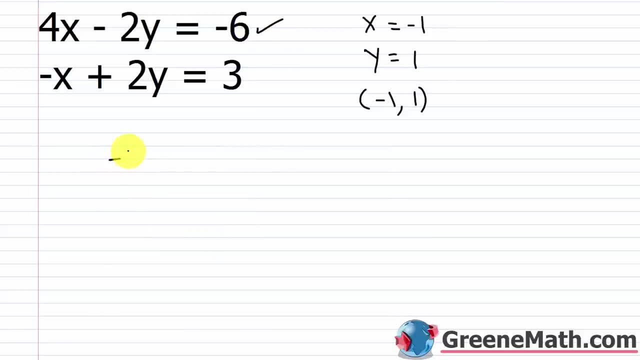 a look at the second one. So I have negative x, So negative plug in a negative 1.. So minus a negative 1 again is plus 1.. Plus 2 times plug in a 1 for y equals 3.. So essentially this would be 1 plus 2. 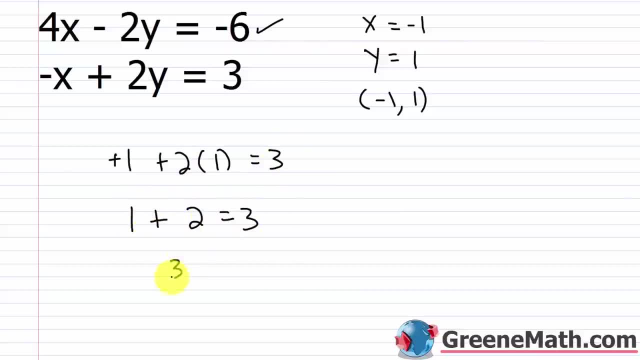 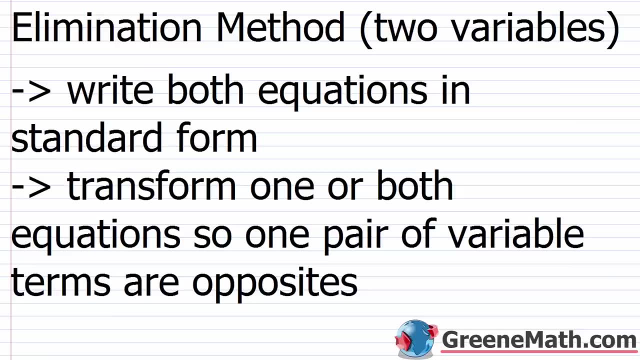 times 1 is 2 equals 3.. We know 1 plus 2 is 3.. We get 3 equals 3.. So it checks out there As well. So now that we've had a chance to look at two very easy examples, let's cover kind of the. 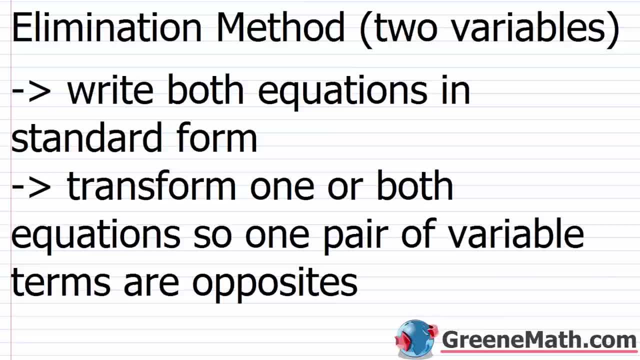 textbook elimination method procedure. So the elimination method for two variables, and obviously this would be with two equations. We want to write both equations in standard form, So ax plus by equals c, And if you want to use the stricter definition, that's fine, You don't need to You. 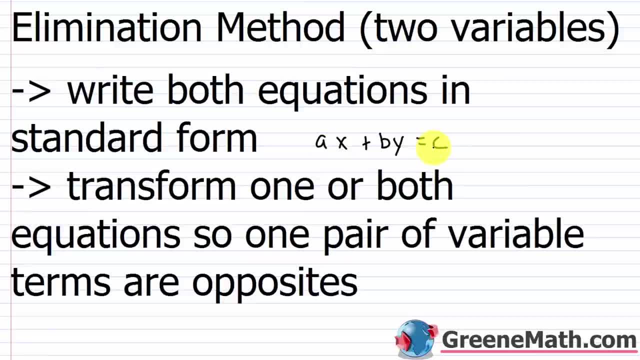 can just have a, b and c as real numbers, Where, as long as you don't have a, b and c as real numbers, you don't have a and b both equal to 0. you would be fine. The next step, and we really haven't. 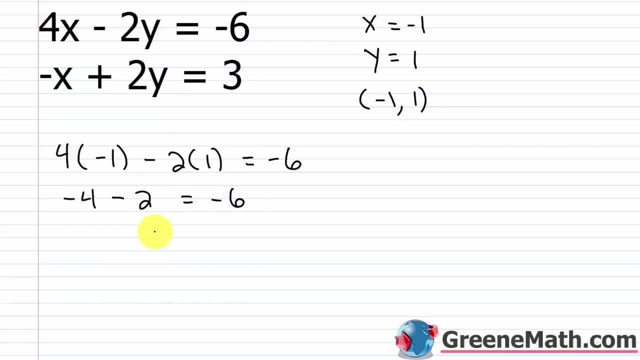 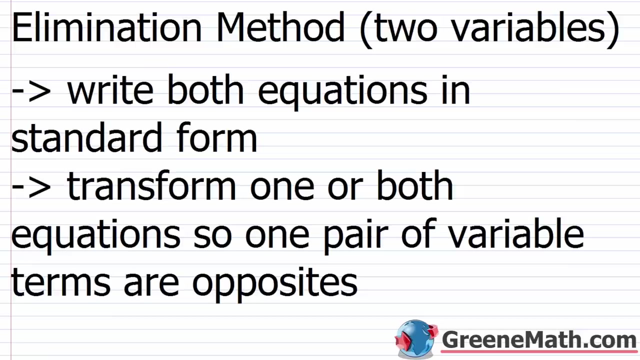 2 equals negative 6 negative 4 minus 2 is negative 6 so you get negative 6 equals negative 6 so it checks out in the first one let's take a look at the second one so i have negative x so negative plug in a negative 1 so minus the negative 1 again is plus 1 plus 2 times plug in a 1 for y equals 3 so essentially this would be 1 plus 2 times 1 is 2 equals 3 we know 1 plus 2 is 3 we get 3 equals 3 so it checks out there as well so now that we've had a chance to look at two very easy examples let's cover kind of the textbook elimination method procedure so the elimination method for two variables and obviously this would be with two equations we want to write both equations in standard form so ax plus by equals c and if you want to use the stricter definition that's fine you don't need to you can just have a b and c as real numbers where as long as you don't have a and b both equal to 0 you'd be fine the next step and we really haven't gotten to this yet because we haven't looked at any difficult problems we want to transform one or both equations so one pair of variable terms are opposites and we're going to see this in a minute in the examples we've looked at we've come into easier problems where we've started out with one pair of variable terms that were opposites So we didn't need to do this step. 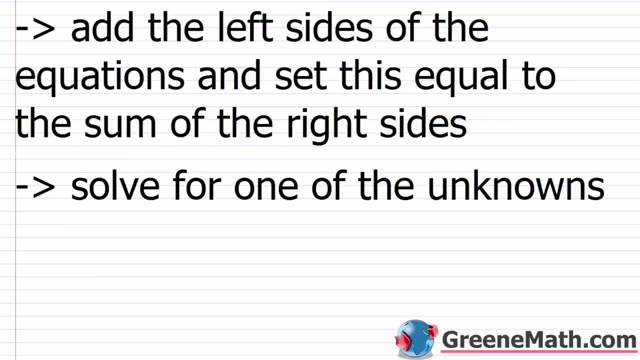 So once this is accomplished, we want to add the left sides of the equations and set this equal to the sum of the right sides. 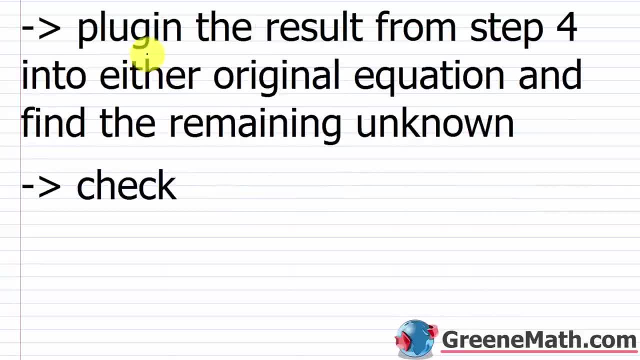 Then we're going to solve for one of the unknowns. We're then going to plug in the result from step 4 into either original equation and find the remaining unknown. 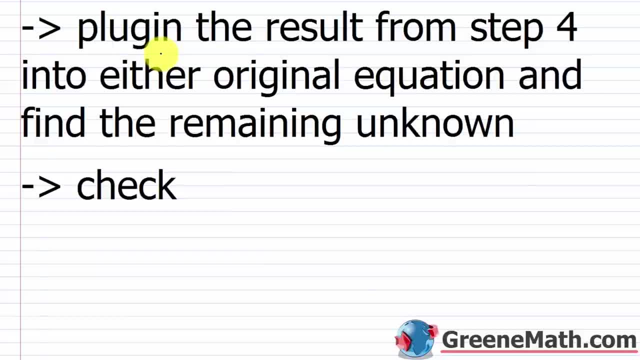 And then we're going to check our solution in each original equation. All right, let's take a look at one that's a little bit harder. 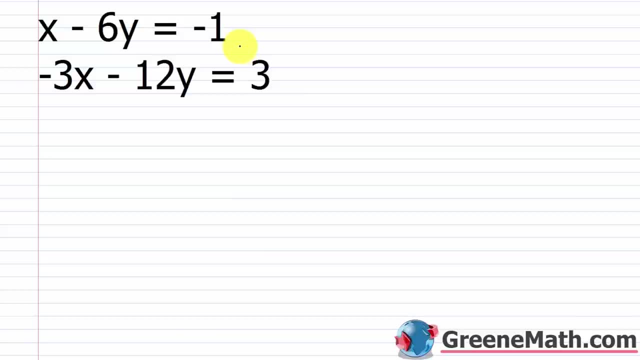 So we have x minus 6y equals negative 1, and negative 3x minus 12y equals 3. So if we look here, we see that they're both in standard form already. ax plus by equals c. 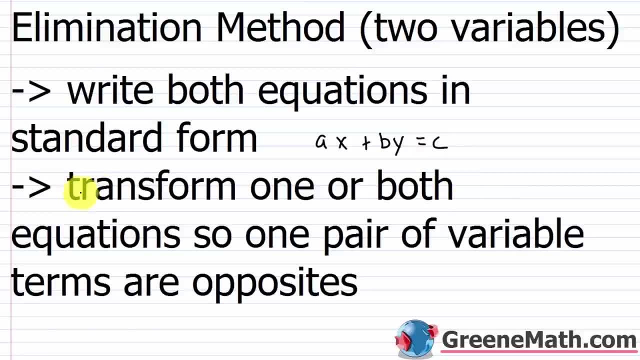 gotten to this yet because we haven't looked at any difficult problems. We want to transform one or both equations, So one pair of variable terms are opposites, And we're going to see this in a minute. In the examples we've looked at we've come into easier problems where we've started out with. 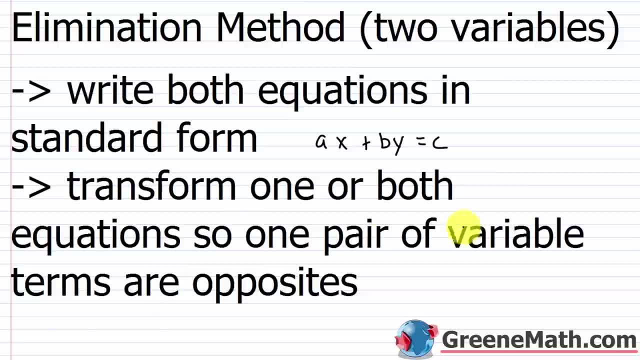 one pair of variable terms that were opposites, So we didn't need to do this step. So one pair of variable terms are opposites, So we didn't need to do this step. So one pair of variable terms are opposites, So we didn't need to do this step. So we didn't need to do this step. So we didn't need to do this step. 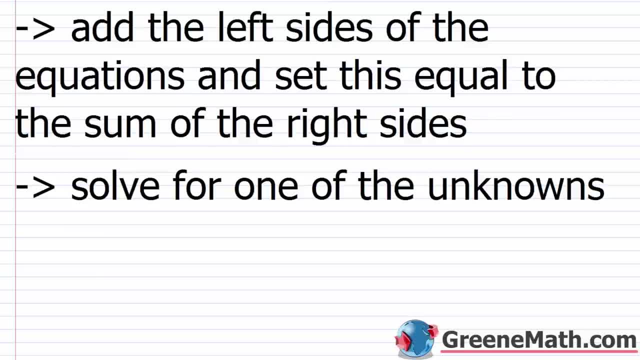 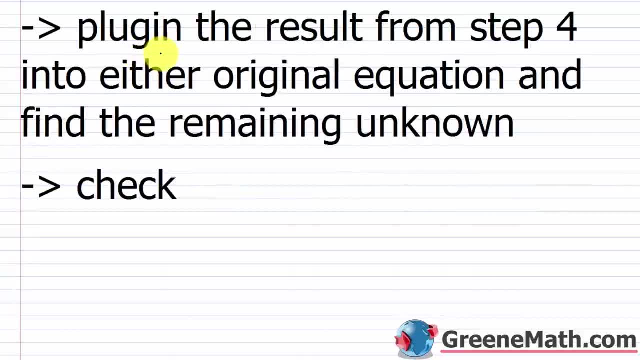 So once this is accomplished, we want to add the left sides of the equations and set this equal to the sum of the right sides. Then we're going to solve for one of the unknowns. We're then going to plug in the result from step 4 into either original equation and find the remaining unknown. 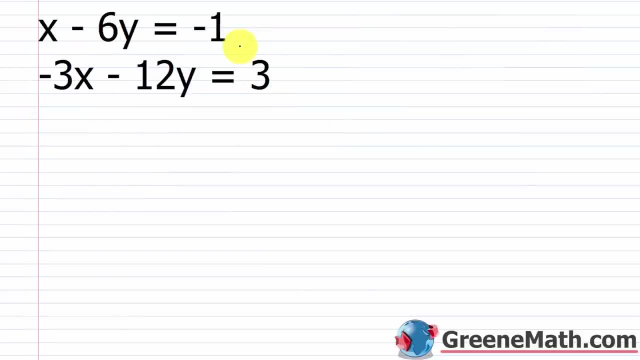 And then we're going to check our solution in each original equation. Alright, let's take a look at one that's a little bit harder. So we have x minus 6y equals negative 1 and negative. 3x minus 12y equals 3.. 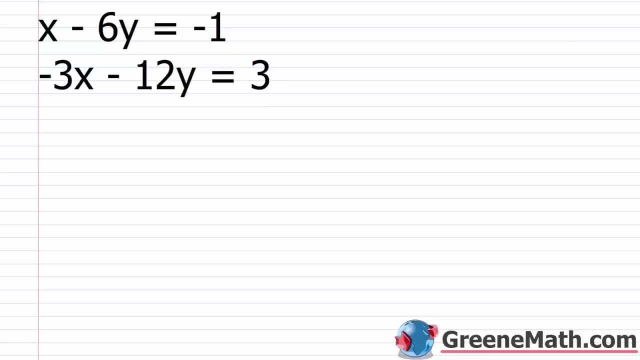 If we look here, we see that they're both in standard form already: ax plus by equals c. The next thing we want to think about is looking at the coefficients for each variable. If I look at the coefficients for x, I have a coefficient here of 1 and a coefficient here of negative 3.. 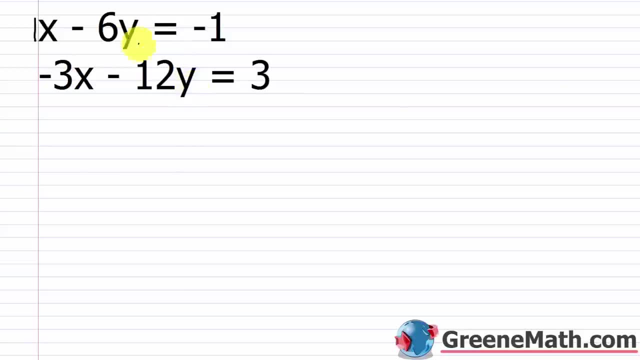 So those aren't opposites. If I look at the coefficients for y, I have negative 6 and negative 12. Those aren't opposites. So I've got to transform one of these two. I've got to transform one or possibly both of the equations into equivalent equations where one pair of variable terms would have opposite coefficients. 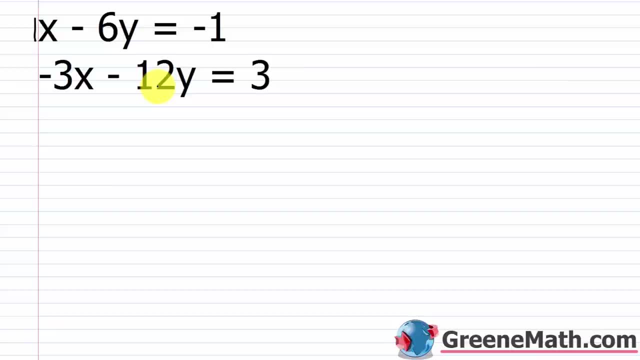 So kind of the easiest thing I can think of right now. if I look at negative 3 here, well, all I would have to do is multiply this equation here both sides, by 3, and what that would do is that would give me a 3x here instead of 1x. 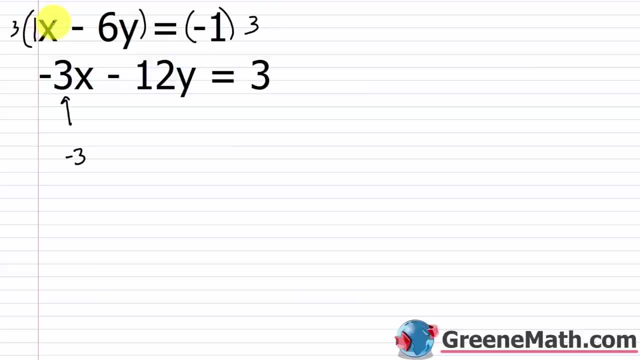 Perfectly legal, because I can multiply both sides by 3.. Perfectly legal, because I can multiply both sides by 3.. Perfectly legal, because I can multiply both sides of an equation by the same number, as long as it's not 0, and I preserve my solution. 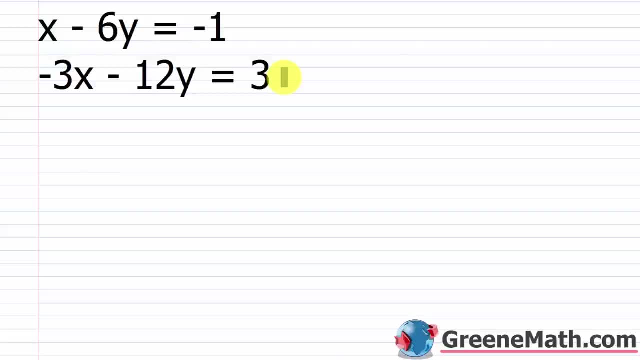 The next thing we want to think about is looking at the coefficients for each variable. If I look at the coefficients for x, I have a coefficient here of 1 and a coefficient here of negative 3. So those aren't opposites. If I look at the coefficients for x, I have a coefficient here of 1 and a coefficient for y, I have negative 6 and negative 12. Those aren't opposites. So I've got to transform one or possibly both of the equations into equivalent equations where one pair of variable terms would have opposite coefficients. 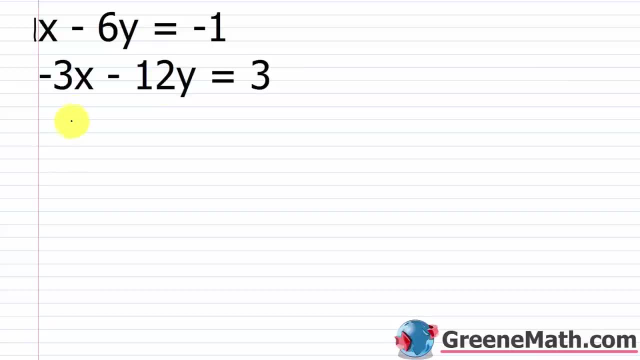 So kind of the easiest thing I can think of right now, if I look at negative 3 here, well, all I would have to do is multiply this equation here, both sides by 3, and what that would do is that would give me a 3x here instead of 1x. Perfectly legal because I can multiply both sides of an equation by the same number, as long as it's not 0, and I preserve my solution. So let me just do that down here. I'm going to drag this guy down here, and I'm going to multiply both sides by 3. So I'm going to do that here. 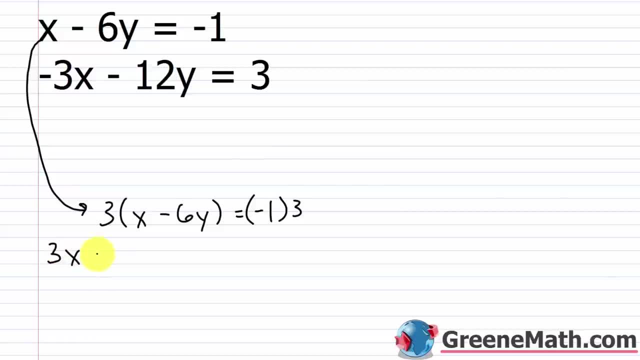 3 times x is 3x, minus 3 times 6y, that's 18y. This equals negative 1 times 3, which is negative 3. 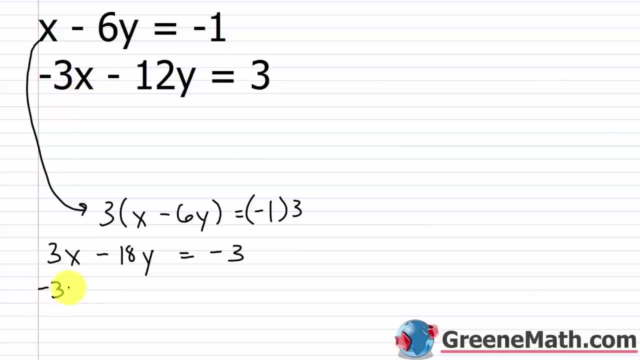 So then here, I'm just going to copy this equation, negative 3x minus 12y equals 3. 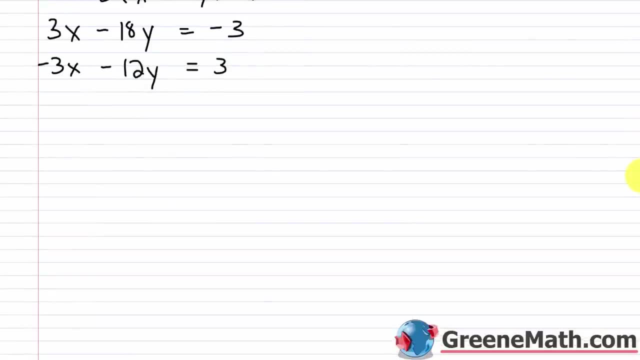 So once we've transformed this equation such that we have a pair of variable terms that have opposite coefficients, we can go through and do our add the left sides together, set that equal to the sum of the right sides. So I'm just going to add vertically. You can do that by doing this. You can just add going down. 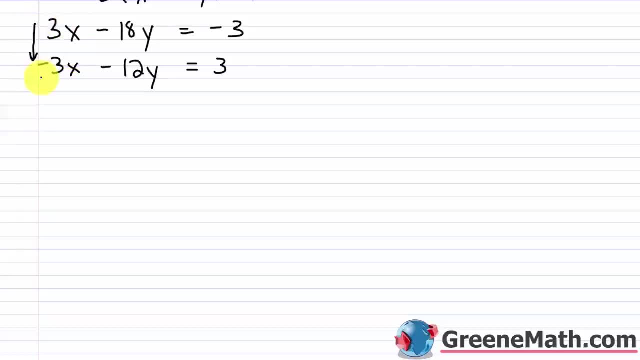 3x plus negative 3x is 0, so this is going to be eliminated. 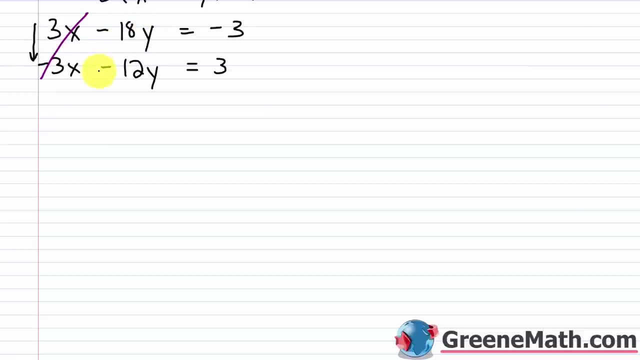 Then the next thing is, we have negative 18y plus negative 12y, 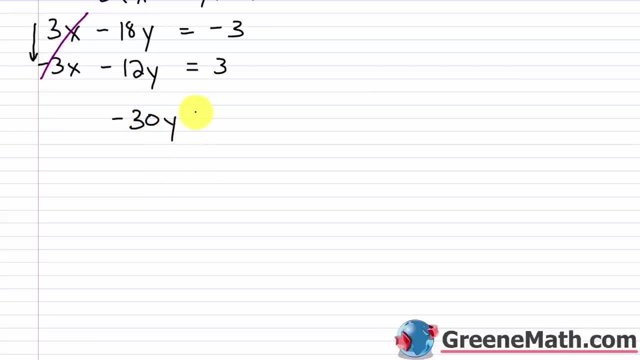 that's negative 30y, and this equals negative 3 plus positive 3, which is 0. Divide both sides of the equation by negative 30, 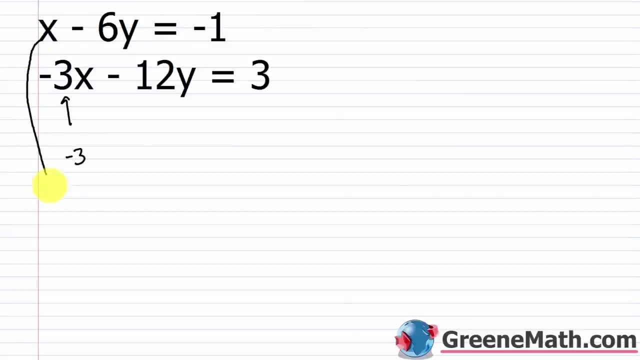 So let me just do that down here. I'm gonna drag this guy down here and I'm going to multiply both sides by 3.. 3 times x is 3x. minus 3 times 6y, that's 18y. This equals negative 1 times 3, which is negative 3.. 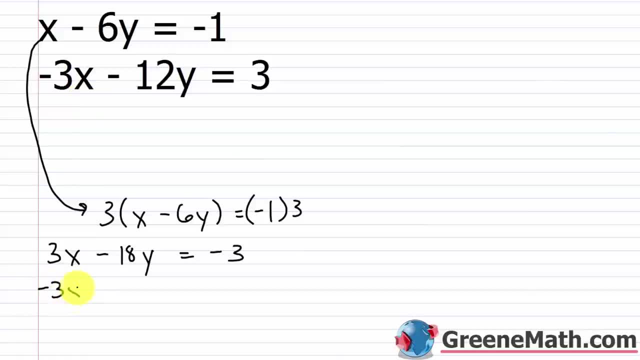 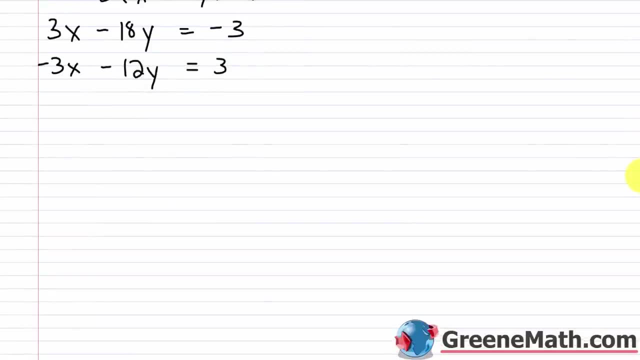 So then here I'm just going to copy this equation: negative 3x minus 12y equals 3.. So once we've transformed this equation such that we have a pair of variable terms that have opposite coefficients, we can go through and do our add the left sides together: set. 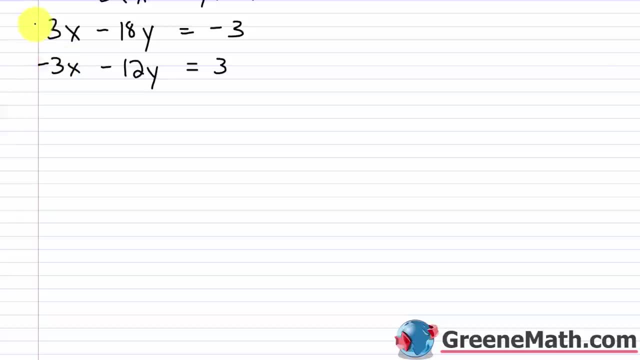 that equal to the sum of the right sides. So I'm just going to add vertically. you can just add: going down: 3x plus negative 3x is 0, so this is going to be eliminated. Then the next thing is we have negative 18y plus negative 12y. that's negative 30y. 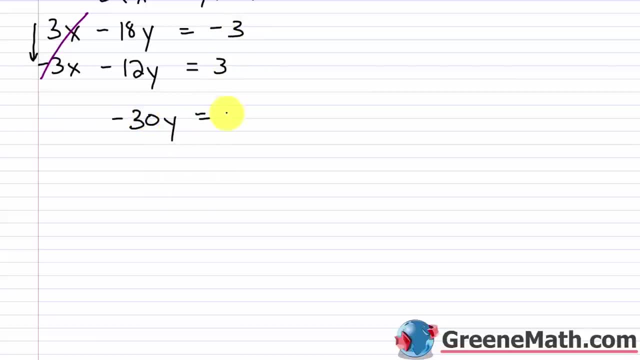 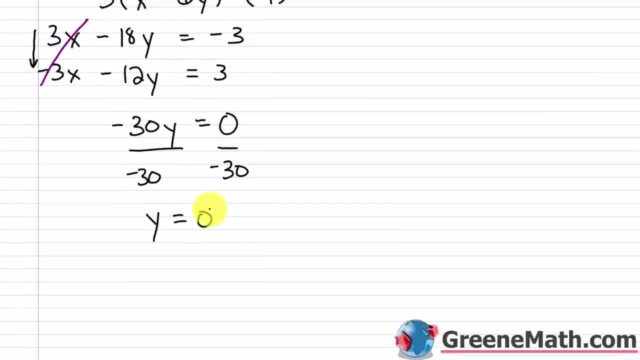 and this equals negative 3 plus positive 3, which is 0.. Divide both sides of the equation by negative 30, and you get that y is equal to 0.. Alright, so we know that y is equal to 0, and again, once I have that information, I 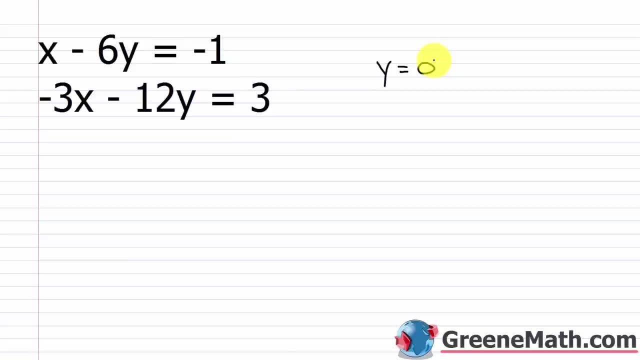 can plug that back in for y in either original equation, It doesn't matter, It doesn't matter which one, So let's go ahead and plug it into the first one. So I would have x minus 6 times 0, just plugged in a 0 for y equals negative 1.. 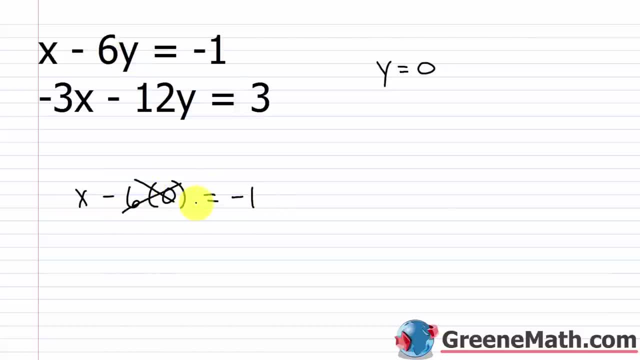 So we know that 6 times 0 is 0, so I can just kind of cross this out and I would have: x is equal to negative 1.. So x is equal to negative 1, so that's the order pair: negative 1 comma 0. 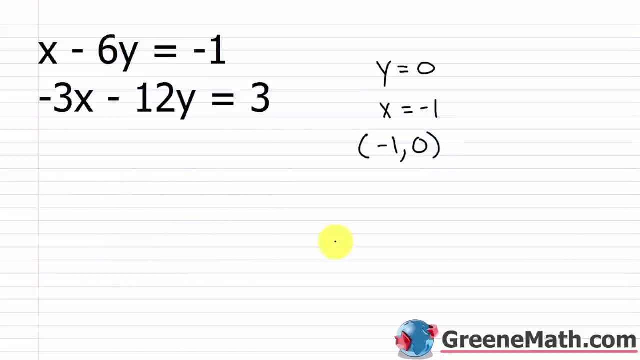 So let's check our result in each original equation. make sure that we didn't make a mistake. So I'd have negative 1 plugged in for x. So I'd have x minus 6 times 0, plug that in for y equals negative 1.. 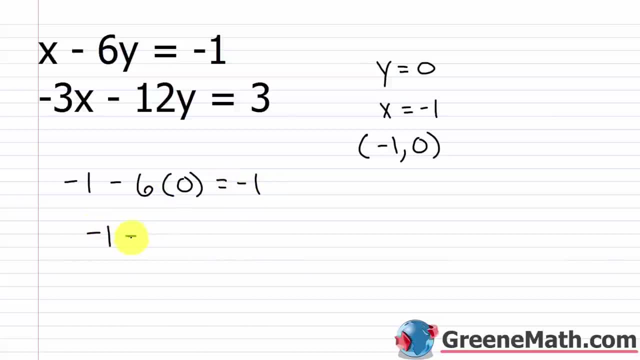 We'd have: negative 1 minus 6 times 0 is 0, so negative 1 minus 0 is just negative 1.. So you get negative 1 is equal to negative 1. So it works out here. Let's take a look at the other one. 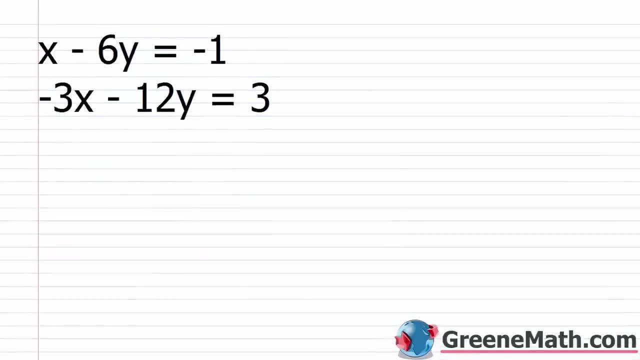 and you get that y is equal to 0. Alright, so we know that y is equal to 0, and again, 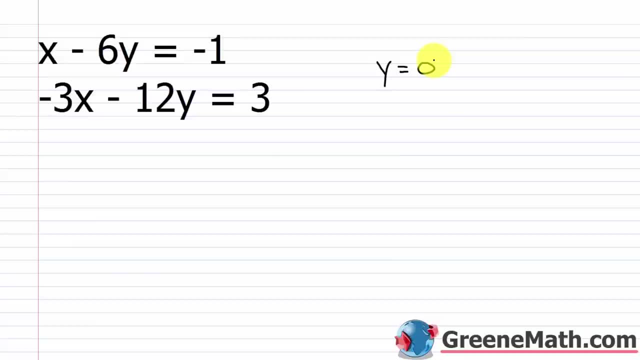 once I have that information, I can plug that back in for y in either original equation. It doesn't matter which one. 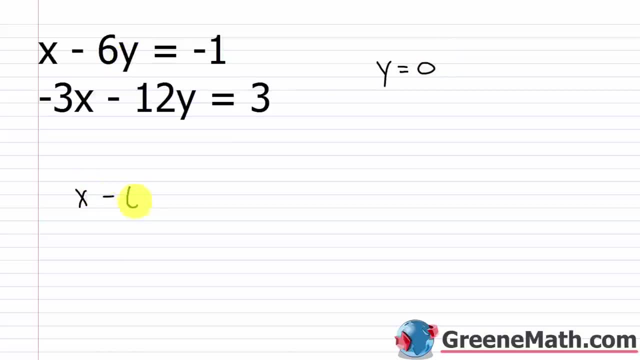 So let's go ahead and plug it into the first one. So I would have x minus 6 times 0, just plugged in a 0 for y, equals negative 1. So we know that 6 times 0 is 0, so I can just kind of cross this out, and I would have x is equal to negative 1. 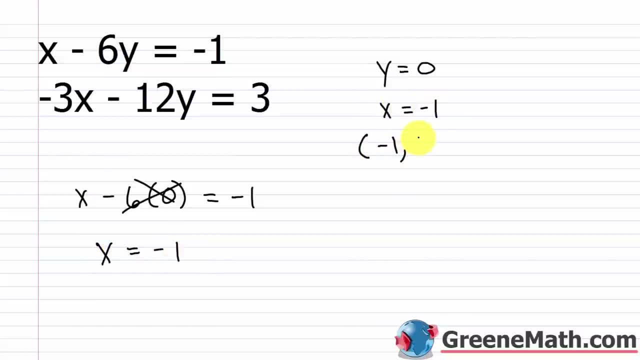 So x is equal to negative 1, so that's the order pair negative 1 comma 0. 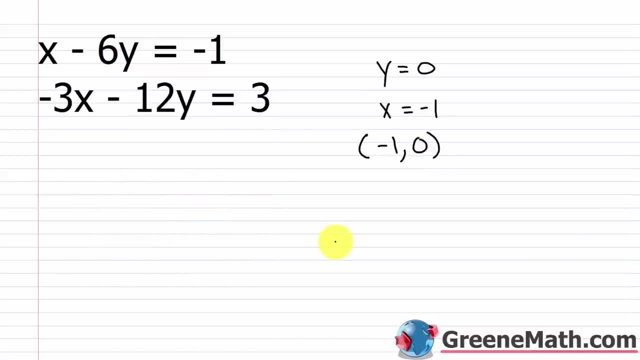 So let's check our result, and each original equation makes sure that we didn't make a mistake. 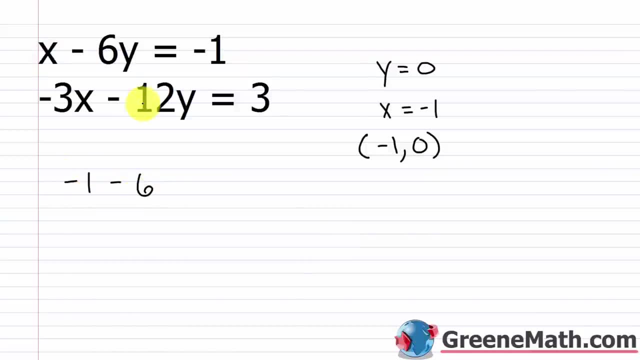 So I'd have negative 1 plugged in for x, minus 6 times 0, plug that in for y, equals negative 1. 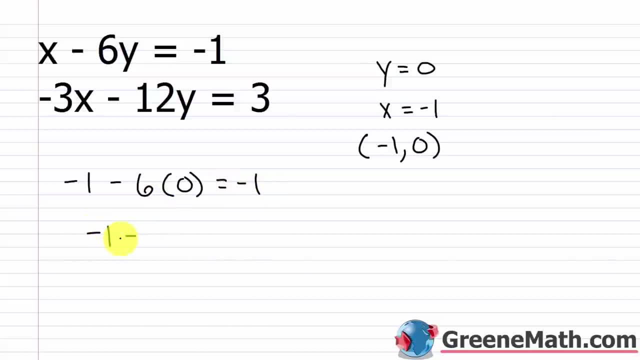 We'd have negative 1 minus 6 times 0 is 0, so negative 1 minus 0 is just negative 1. So you get negative 1 is equal to negative 1. So it works out here. 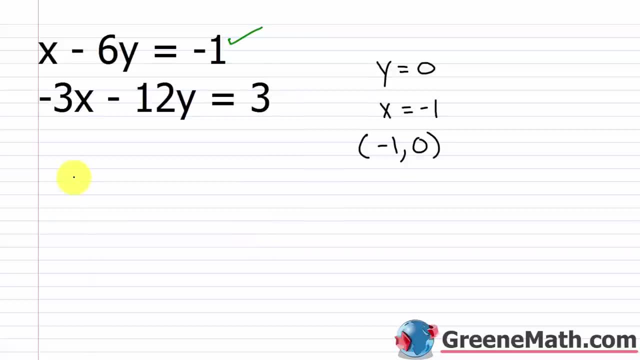 Let's take a look at the other one. We have negative 3x, so negative 3 times negative 1, minus 12y, so minus 12 times 0 equals 3. Negative 3 times negative 1 is positive 3. 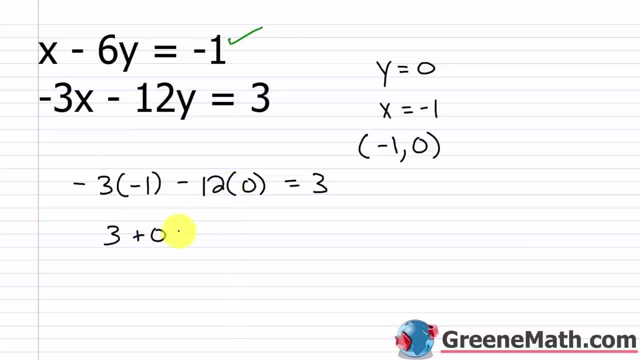 And then negative 12 times 0 is 0, so plus 0 equals 3. You get 3 equals 3. So it works out here as well. 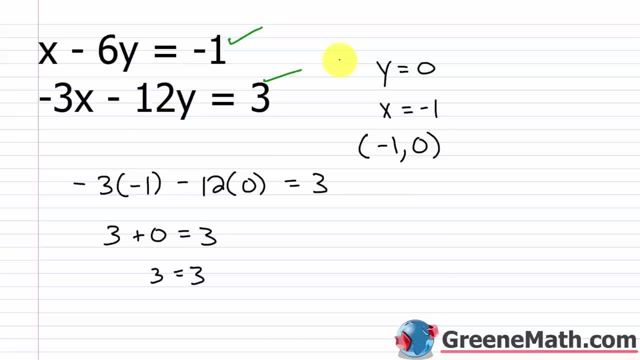 So we've verified that the ordered pair negative 1 comma 0 is the solution for our system. 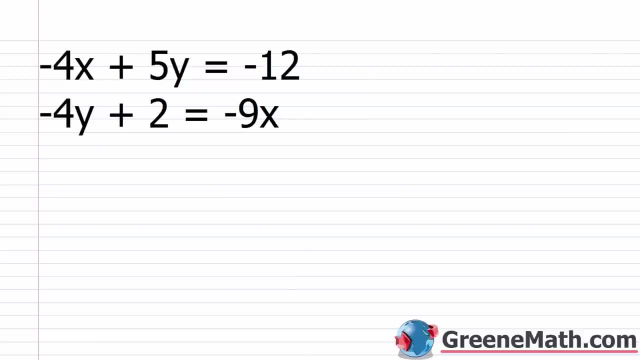 All right, let's look at one that's a little bit more complicated now. I have a negative 4x plus 5y equals negative 12. 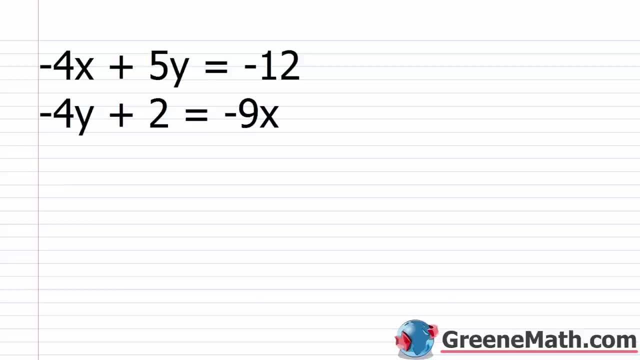 And I have a negative 4y plus 2 equals negative 9x. 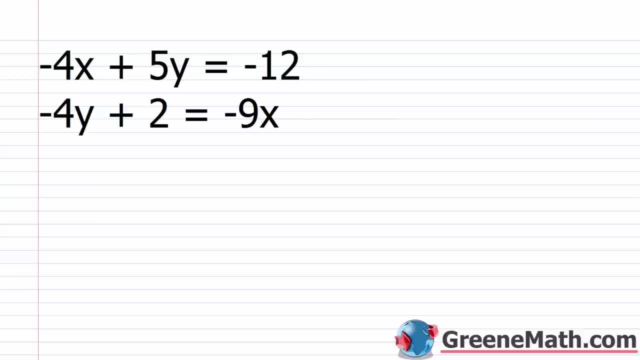 So the first thing that you'll notice is that each equation is not in standard form. 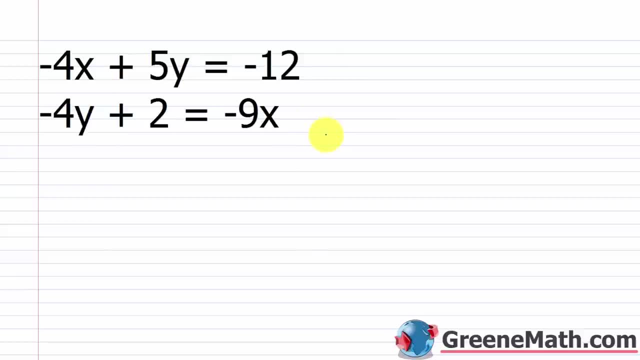 So when you look at it and you try to compare things, it's not easy, and it's a cluster. 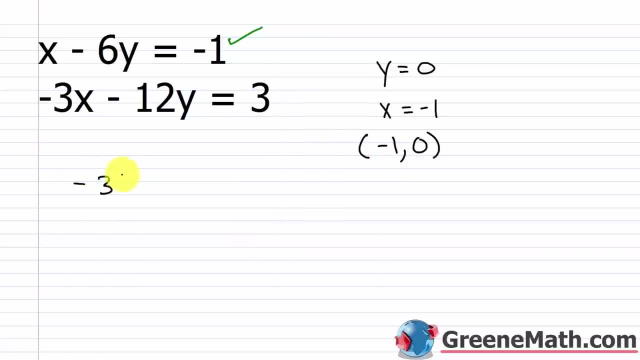 We have negative 3x, so negative 3 times negative. 1, minus 12y, so minus 12 times 0, equals 3.. Negative 3 times 0 equals 3.. Negative 3 times negative: 1 is positive 3, and then negative 12 times 0 is 0,, so plus. 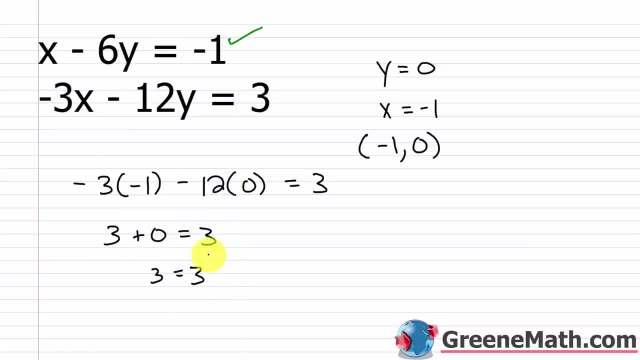 0 equals 3.. You get 3 equals 3, so it works out here as well. So we've verified that the ordered pair- negative 1 comma 0, is the solution for our system. All right, let's look at one that's a little bit more complicated now. 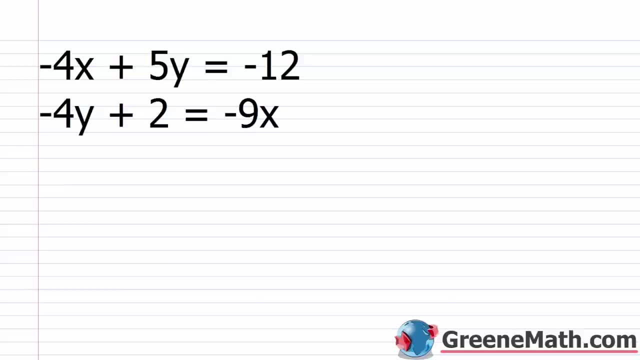 I have negative 4x plus 5y equals negative 12, and I have negative 4y plus 2 equals negative 9x. So the first thing that you'll notice is that I have negative 4y plus 2 equals negative 9x. 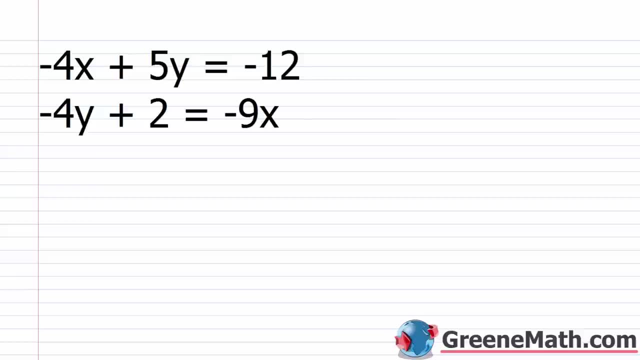 So the first thing that you'll notice is that each equation is not in standard form. So when you look at it and you try to compare things, it's not easy and it's a cluster. So you want to put each equation as ax plus by equals c. 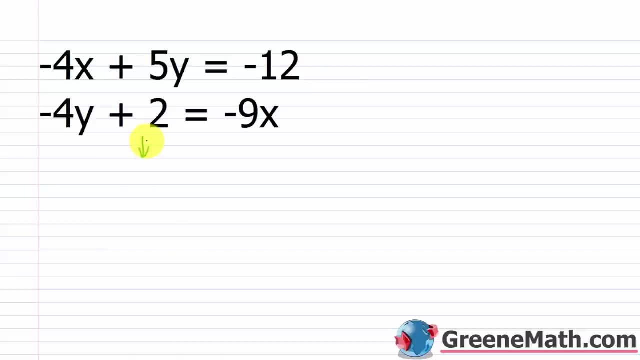 So this one, I'm going to leave alone. This one, I'm just going to move the x variable over here and I'm going to move the constant over here, And I'm just going to do that with the addition property of equality. So I'm going to add 9x to both sides of the equation. 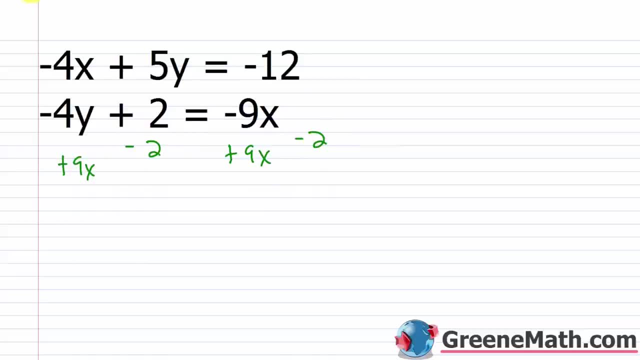 And I'm going to subtract 2 away from each side of the equation. So when the dust settles I'm going to have 9x minus 4y. This will cancel So equals. this will cancel negative 2.. So now we have 9x minus 4y, equals negative 2.. 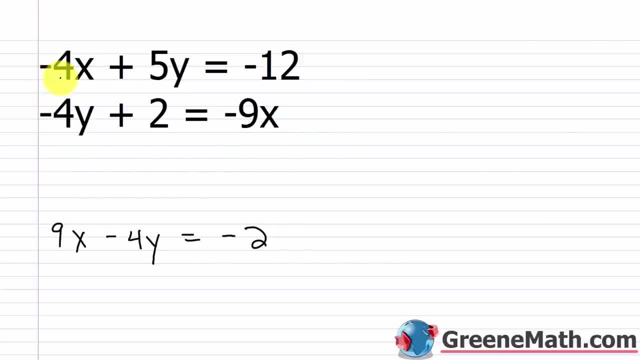 All right. so let's erase this real quick. And I'm just going to drag this other equation down here, so they're on top of each other. So we'll have negative 4x plus negative 12.. Plus 5y equals negative 12.. 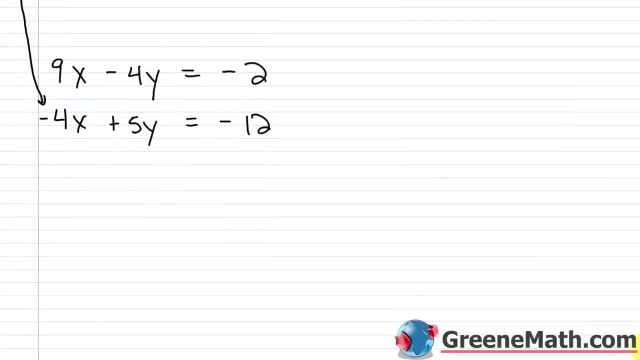 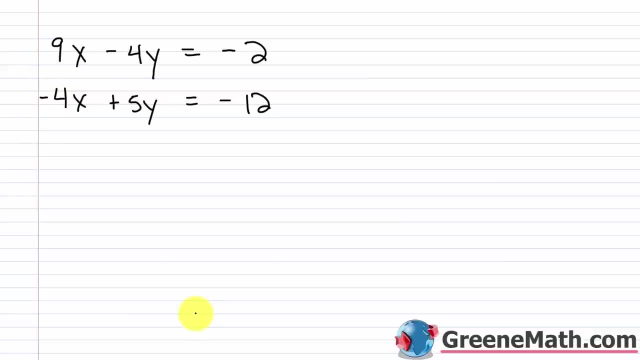 Okay, so now that the first step is completed and they're both in standard form, the next thing that I want to do is I want to look at the coefficients on my variables. So for the x variable, I have a 9 and I have a negative 4.. 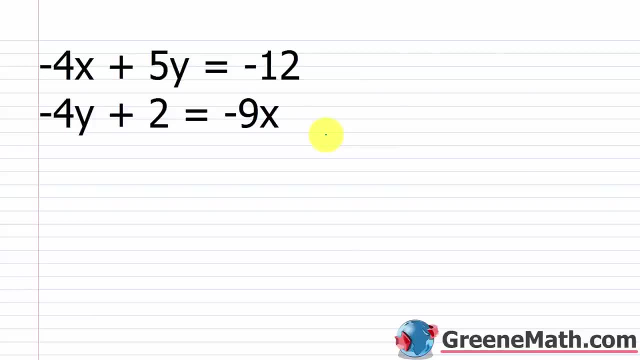 So you want to put each equation as ax plus by equals c. So this one I'm going to leave alone. 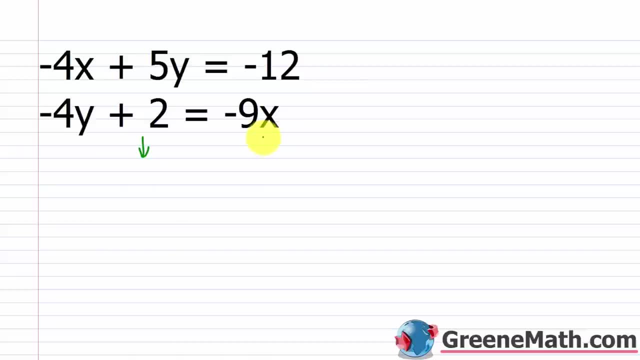 This one I'm just going to move the x variable over here, and I'm going to move the constant over here. And I'm just going to move the constant over here. 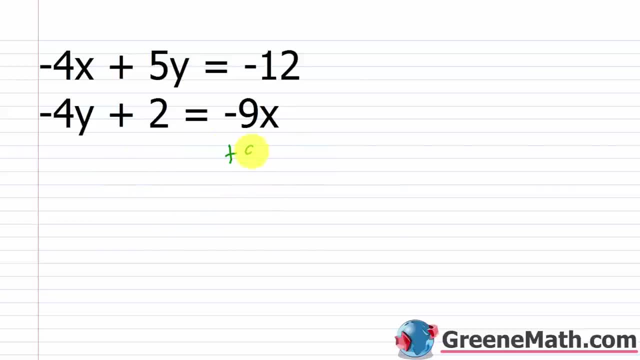 So I'm just going to do that with the addition property of equality. So I'm going to add 9x to both sides of the equation, and I'm going to subtract 2 away from each side of the equation. So when the dust settles, I'm going to have 9x minus 4y. This will cancel. So equals, this will cancel, negative 2. So now we have 9x minus 4y equals negative 2. 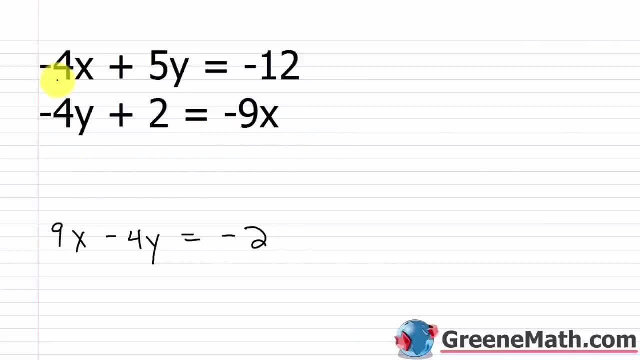 All right, so let's erase this real quick. And I'm just going to drag this other equation over here, and I'm just going to drag this other equation down here. So they're on top of each other. 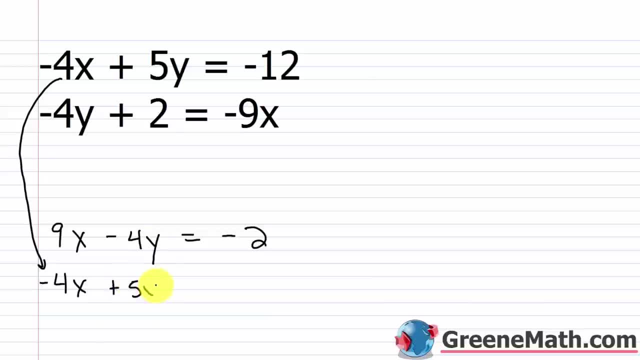 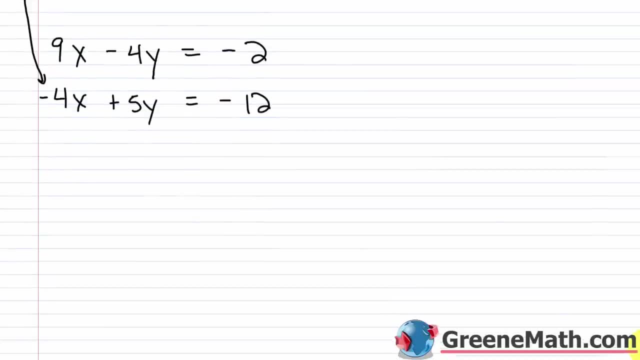 So I have negative 4x plus 5y equals negative 12. Okay, so now that the first step is completed, and they're both in standard form, the next thing that I want to do is I want to look at the coefficients on my variables. So for the x variable, I have a 9, and I have a negative 4. For the y variable, I have a negative 4, and I have a 5. So I don't have anything with, opposite coefficients, so nothing would cancel right now if I did the addition. 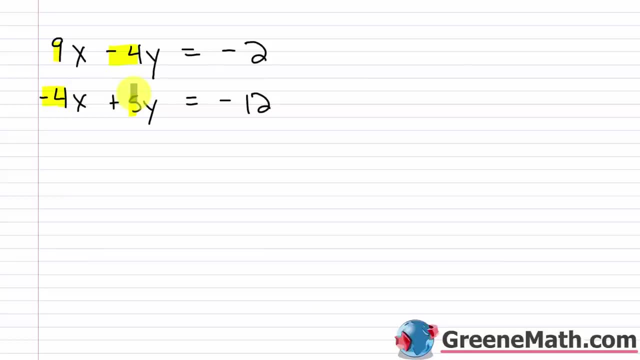 So I've got to transform one or both equations to where one of the variables would drop out. Now it doesn't matter which one you pick. I could pick the x variable and eliminate it, or I could pick the y variable, doesn't matter. 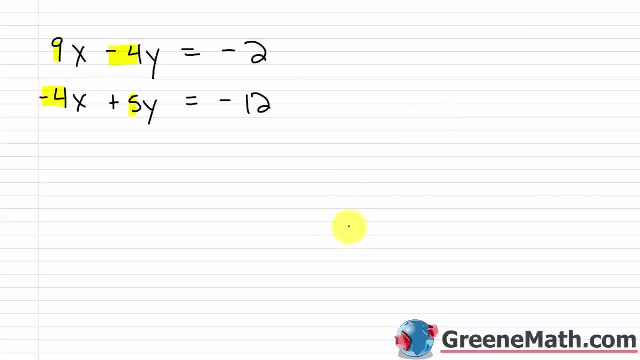 Let's go ahead and work with the x variable. So I have a coefficient here that's 9. I have a coefficient here that's negative 4. So one of them is positive. One of them is negative. So kind of the easy thing to do is just multiply both sides of the first equation by 4, right? That would give me 36 here, or a 36x. 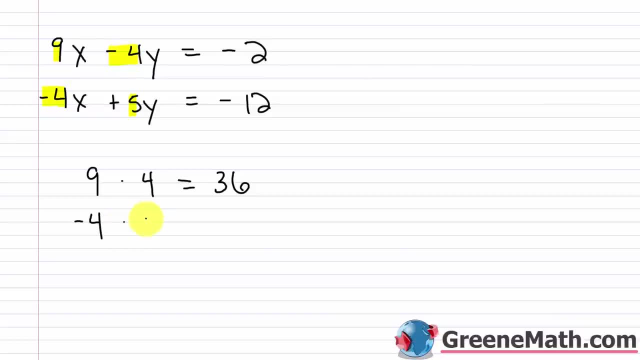 And then multiply both sides of the kind of second equation by 9. That would give me a negative 36x, right? 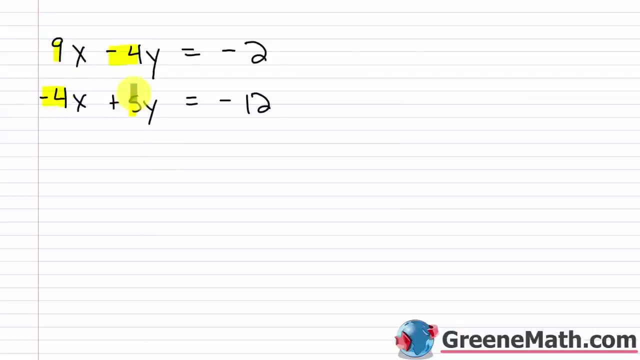 For the y variable. I have a negative 4 and I have a 5. So I don't have anything with opposite coefficients. so nothing would cancel right now if I did the addition. So I've got to transform one or both equations to where one of the variables would drop out. 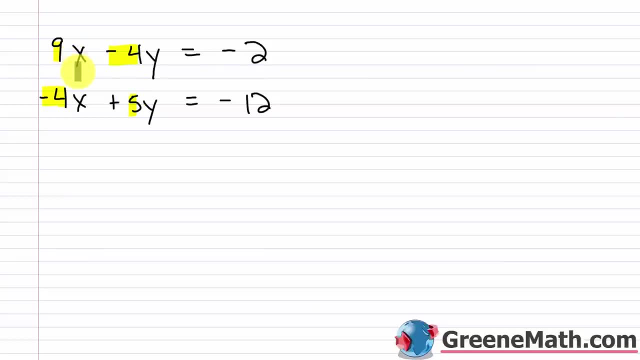 Now, it doesn't matter which one you pick. I could pick the x variable and eliminate it, or I could pick the y variable. doesn't matter, Let's go ahead and work with the x variable. So I have a coefficient here. that's 9.. 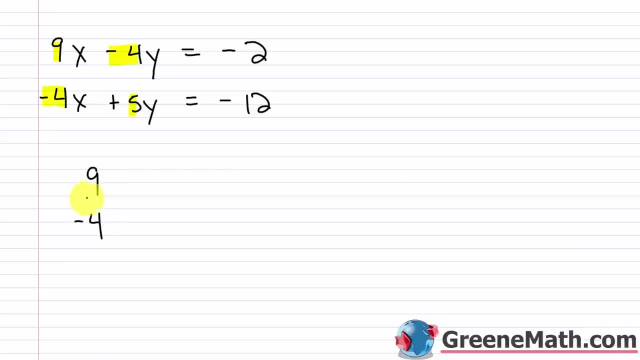 I have a coefficient here that's negative, 4.. So one of them is positive, one of them is negative. So kind of the easy thing to do is just multiply both sides of the first. So let's do it again here. So when I multiply the first equation by 4, that would give me 36 here, or 36x, and then 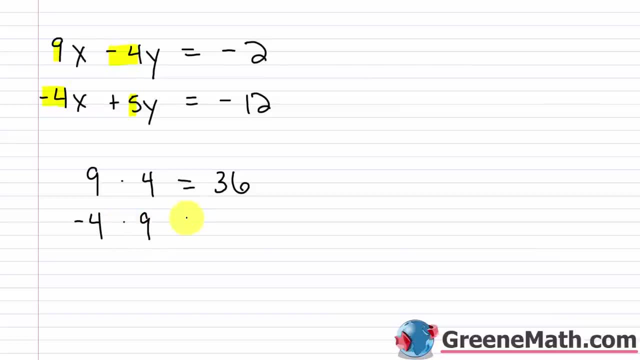 multiply both sides of the second equation by 9, that would give me a negative 36x. So let's go ahead and make that happen. We'll multiply both sides of this equation by 4.. Let me scooch this over a little bit. 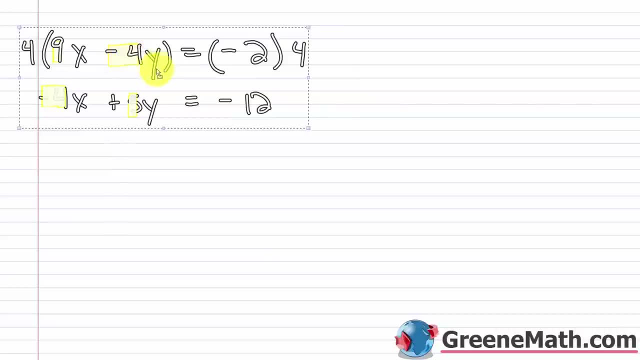 And let's see what happens. Okay, Let's multiply both sides of this equation by 9.. So, for the first equation, 4 times 9x is 36x minus 4 times 4y, which is 16y, and this equals. 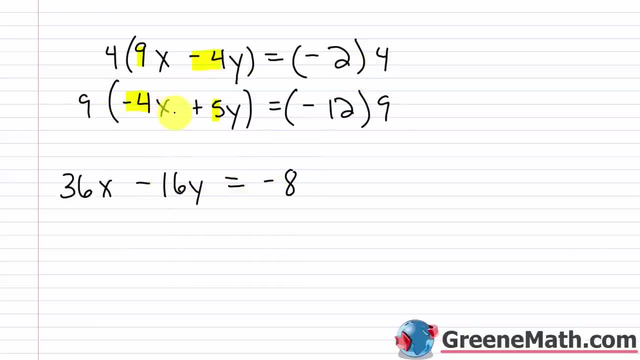 negative 2 times 4,, which is negative 8.. Then we have 9 times negative 4x, that's negative 36x. 9 times 5y, that's going to be plus 45y. This equals 9 times negative 12, which is negative 180. 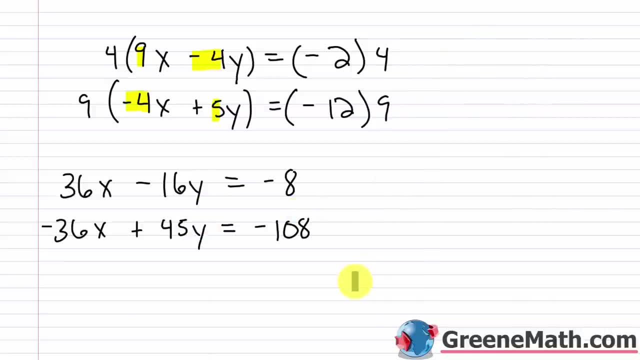 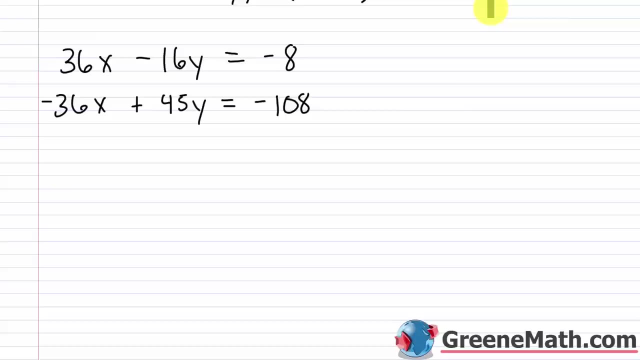 So now that we have transformed both of the equations into equivalent equations where through the addition process, this variable x would be eliminated, right, you have opposite coefficients here, 36 and negative 36.. We can go through and do that addition step now. 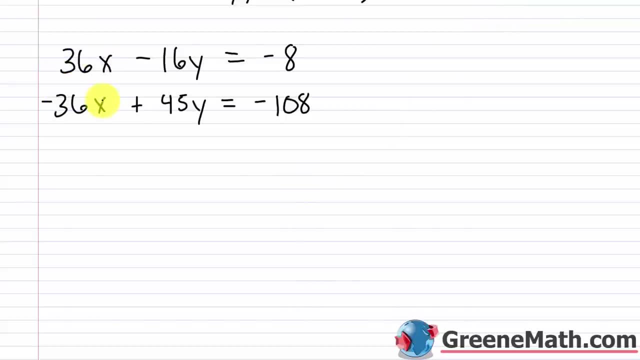 So we're going to add the two left sides together, so 36x plus negative 36x, that's zero. so this is the limit. negative 16y plus 45y is 29y. This is equal to negative 8 plus negative 108,, which is negative. So let's go ahead and make that happen. 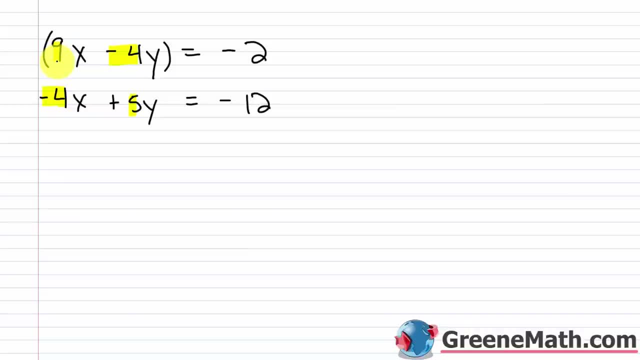 We'll multiply both sides of this equation by 4. Let me scooch this over a little bit. 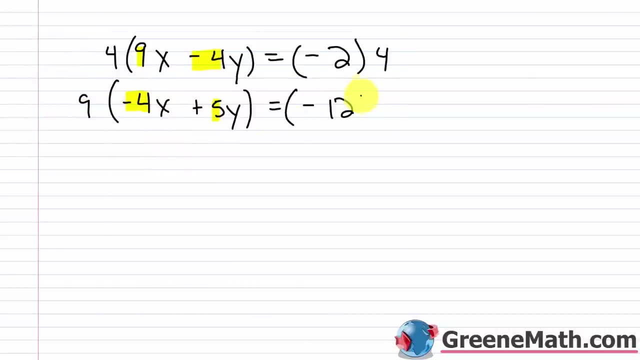 And let's multiply both sides of this equation by 9. So for the first equation, 4 times 9x is 36x, minus 4 times 4y, which is 16y. And this equals negative 2 times 4, which is negative 8. 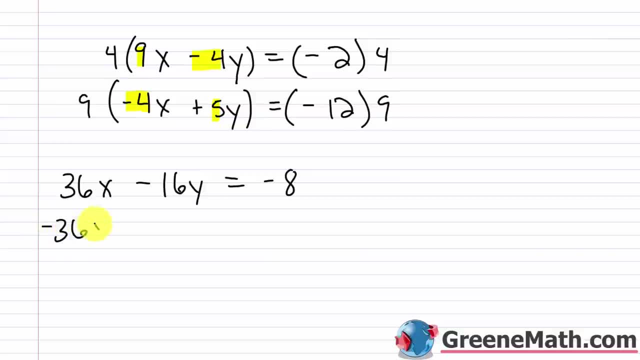 Then we have 9 times negative 4x, that's negative 36x. 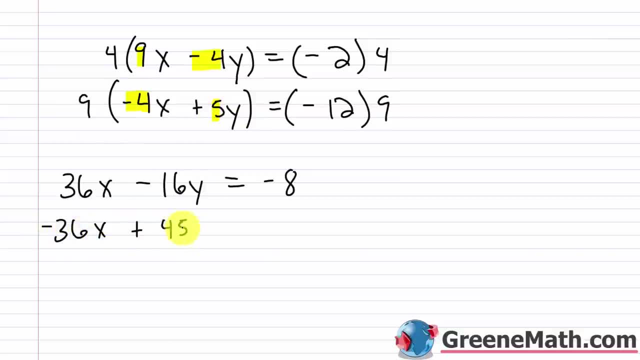 9 times 5y, that's going to be plus 45y. 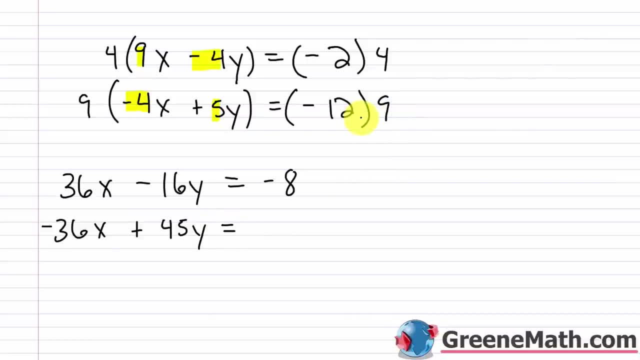 This equals 9 times negative 12, which is negative 108. All right. 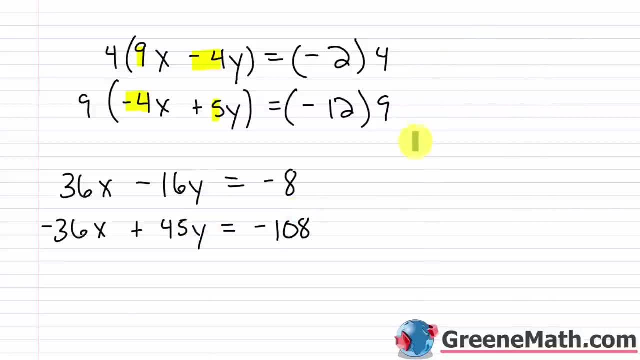 So now that we have transformed both of the equations into equivalent equations where through the addition process, this variable x would be eliminated, right? You have opposite coefficients here, 36 and negative 36. We can go through and do that addition step now. So we're going to add the two left sides together. So 36x plus negative 36x. That's 0x. That's 0x. So this is eliminated. 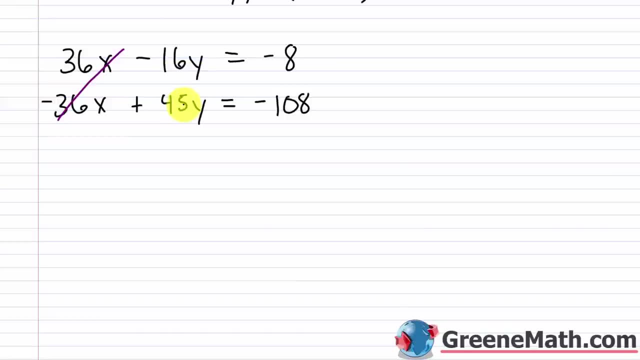 Negative 16y plus 45y is 29y. 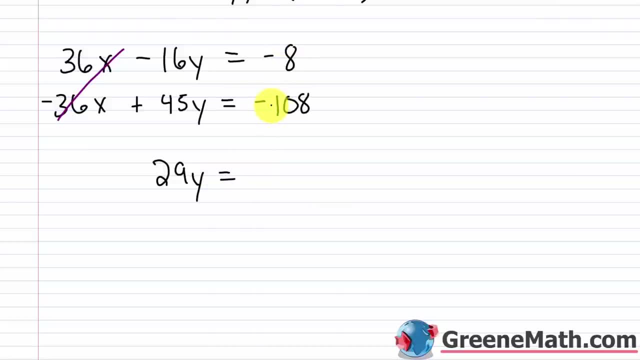 This is equal to negative 8 plus negative 108, which is negative 116. 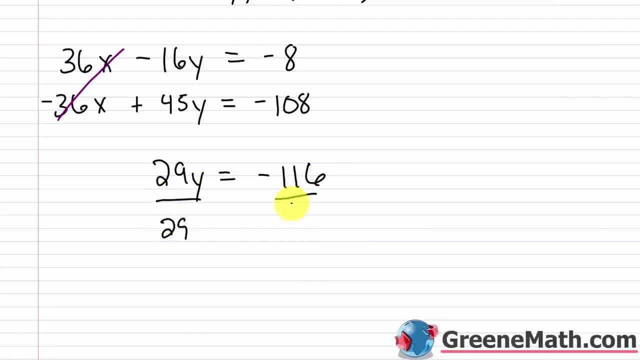 Now, if I divide both sides of the equation by 29, the coefficient of y, I'm going to get that y is equal to negative 4. Negative 116 divided by 29 is negative 4. So y is equal to negative 4. So now I can plug a negative 4 in. 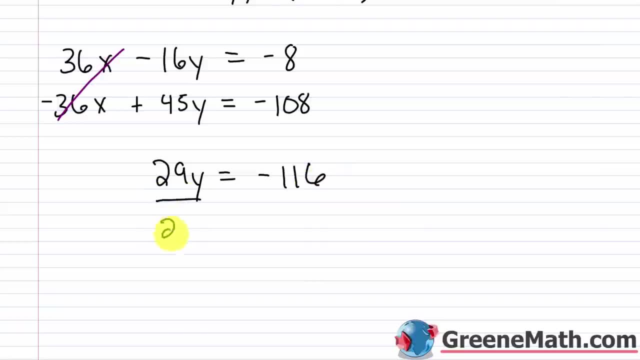 116.. Now if I divide both sides of the equation by 29, the coefficient of y, I'm going to get that y is equal to negative 4.. Negative 116 divided by 29 is negative 4.. So y is equal to negative 4.. 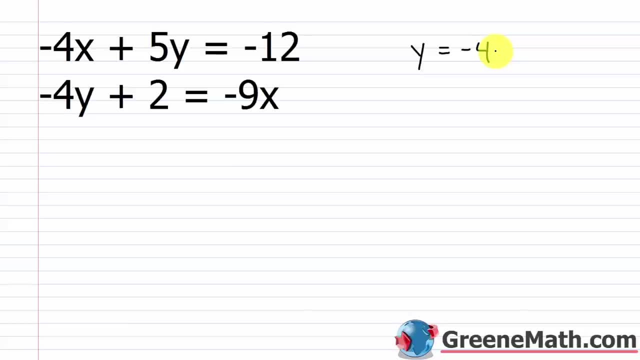 So now I can plug a negative 4 in for y in either original equation. solve for x, So let's go ahead and plug it into the second equation. So we'd have negative 4 times negative. 4 plus 2 equals negative 9x. Negative 4 times negative 4 is 16.. So you'd have 16 plus 2 equals negative 9x, 16 plus. 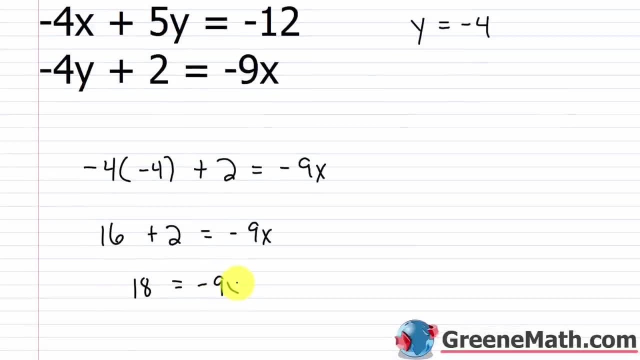 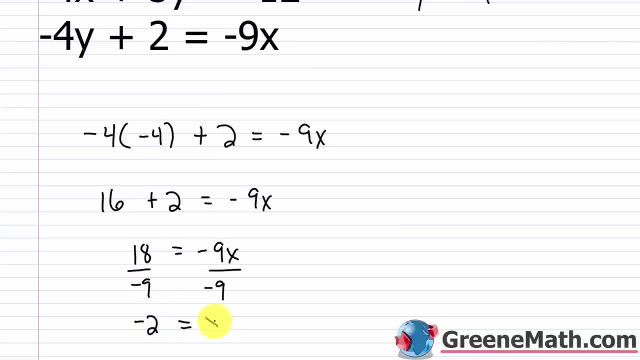 2 is 18.. So you'd have 18 equals negative 9x. Divide both sides of the equation by negative 9.. And you're going to get that negative 2 is equal to x, or you could say x is equal to negative 2.. 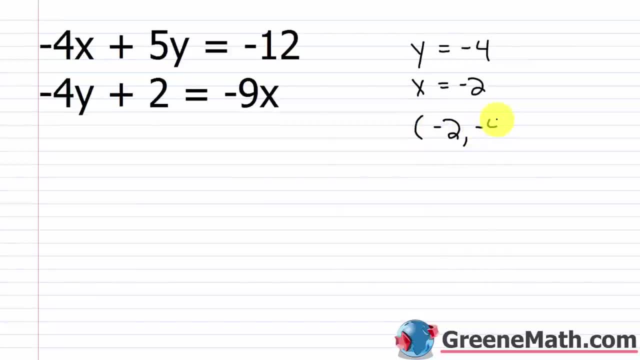 So this would be the ordered pair: negative 2 comma, negative 4.. All right, so let's plug in for x and y in the original equations and make sure that this is the solution for the system. So we'll have negative 4 times. plug in a negative 2 for x, plus 5 times plug in a negative 4 for y. 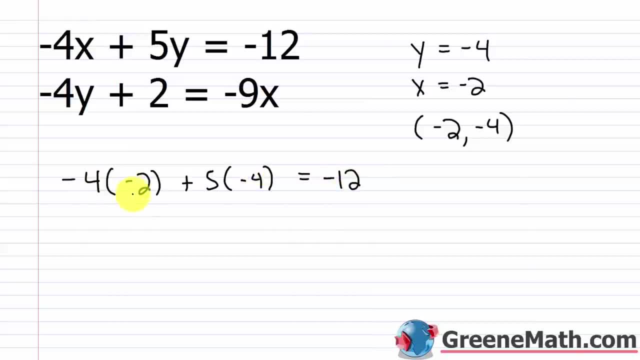 equals negative 12.. Negative 4 times negative 2 is 8.. 5 times negative 4 is negative 20.. So minus 20 equals negative 12. And this is true: 8 minus 20 is negative 12. So you get negative 12 equals. 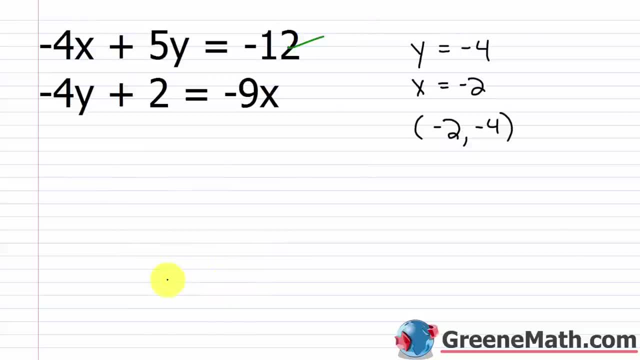 negative 12.. It checks out there. All right. for the next one, we have negative 4y, so negative 4 times for y. I have a negative 4, plus 2 equals negative 9 times negative 2,. plug in a negative 2. 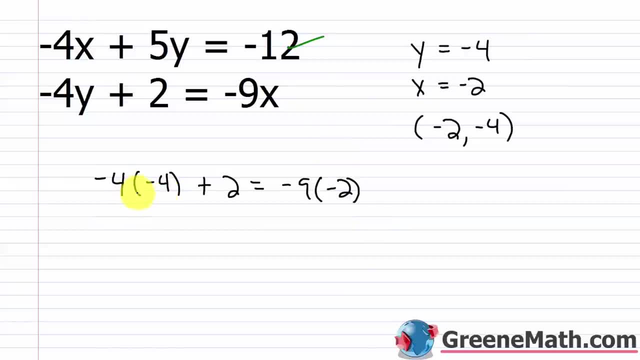 for x, Negative 4 times negative 4 is 16.. So you'd have 16 plus 2, that's 18.. So this equals negative 9 times negative 2, that's 18 also. So it works out here as well. So we've verified that this ordered pair. 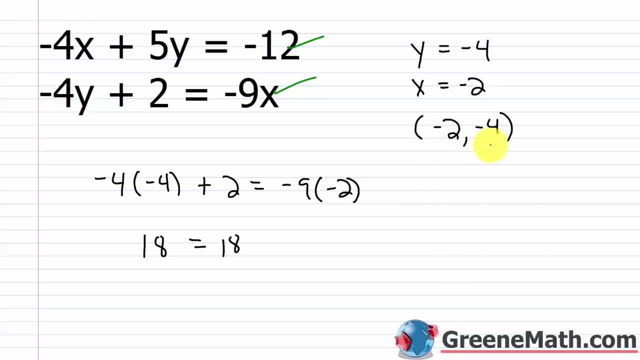 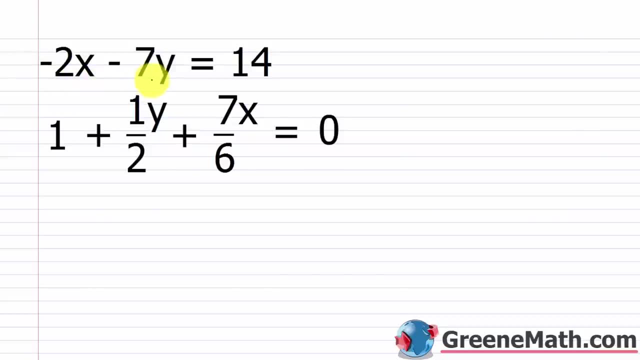 negative 2 comma, negative 4, is the solution for the system. All right, let's take a look at one final problem Again. as you practice this, it becomes very, very easy. We have negative 2x minus 7y equals 14.. And we have 1 plus 1 half y plus 7, 6x equals 0. So this equation is: 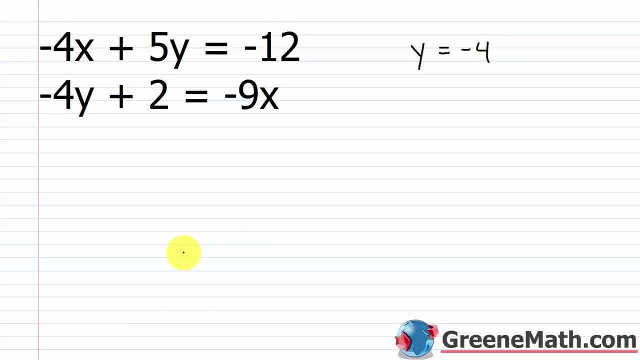 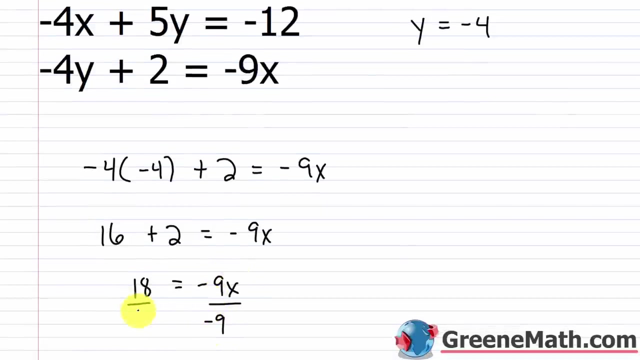 For y in either original equation, solve for x. So let's go ahead and plug it into the second equation. So we'd have negative 4 times negative 4 plus 2 equals negative 9x. Negative 4 times negative 4 is 16. So you'd have 16 plus 2 equals negative 9x. 16 plus 2 is 18. So you'd have 18 equals negative 9x. Divide both sides of the equation by negative 9. 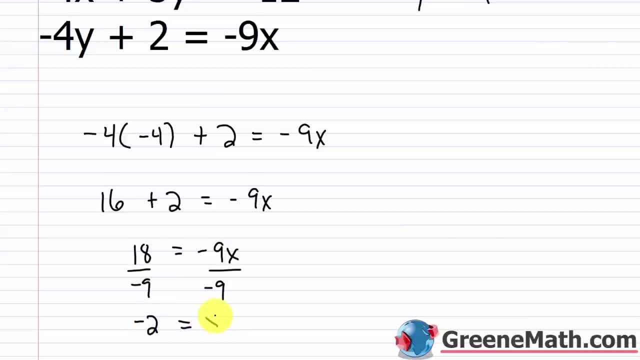 And you're going to get that negative 2 is equal to x. 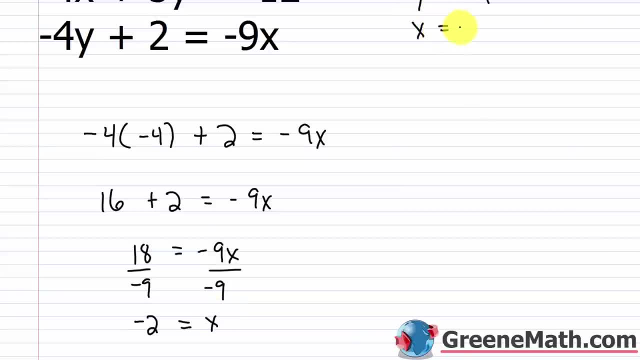 Or you could say x is equal to negative 2. So this would be the ordered pair, negative 2 comma negative 4. 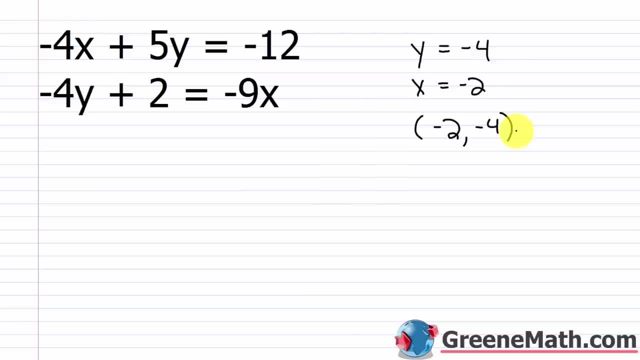 All right, so let's plug in for x and y in the original equations and make sure that this is the solution for the system. 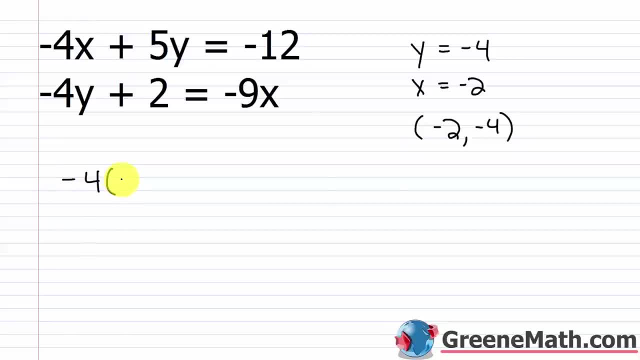 So we'll have negative 4 times, plug in a negative 2 for x, plus 5 times, plug in a negative 4 for y, equals negative 12. Negative 4 times negative 2 is 8. 5 times negative 4 is negative 20. 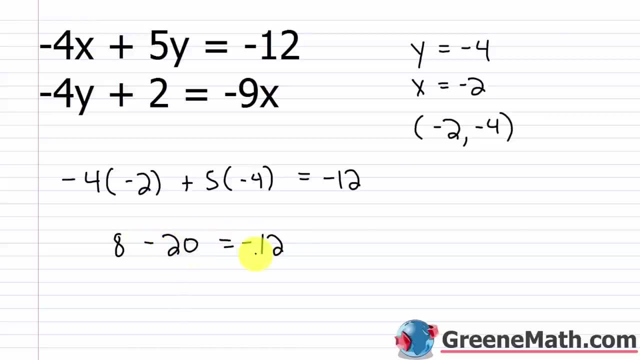 So minus 20 equals negative 12. And this is true. 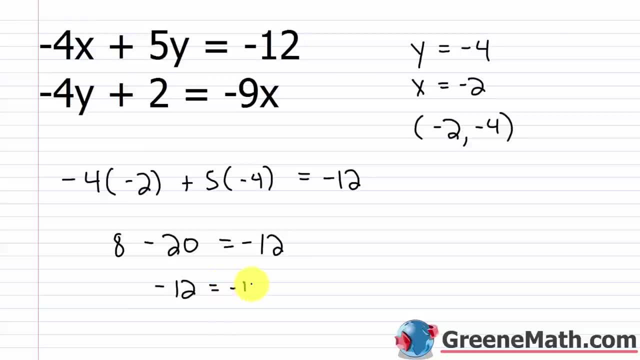 8 minus 20 is negative 12. So you get negative 12 equals negative 12. It checks out there. 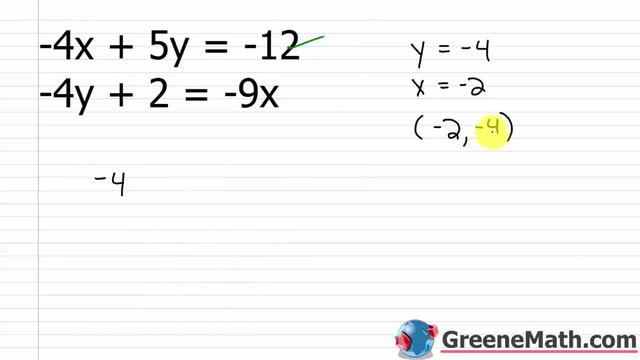 All right, for the next one, we have negative 4y. So negative 4 times, for y I have a negative 4, plus 2 equals negative 9 times negative 2. Plug in a negative 2 for x. 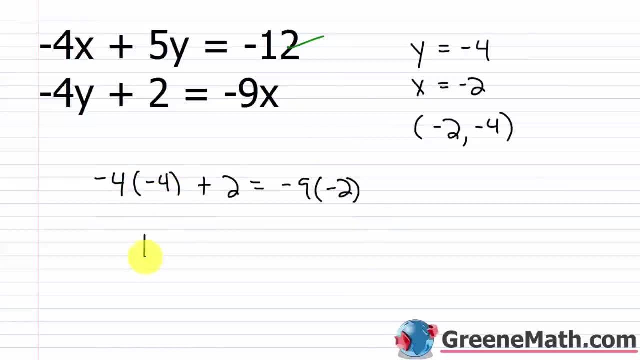 Negative 4 times negative 4 is 16. So you'd have 16 plus 2, that's 18. So this equals negative 9 times negative 2, that's 18 also. So it works out here as well. 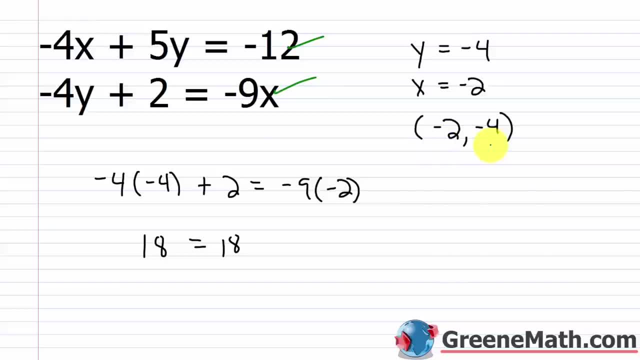 So we've verified that this ordered pair, negative 2 comma negative 4, is the solution for the system. 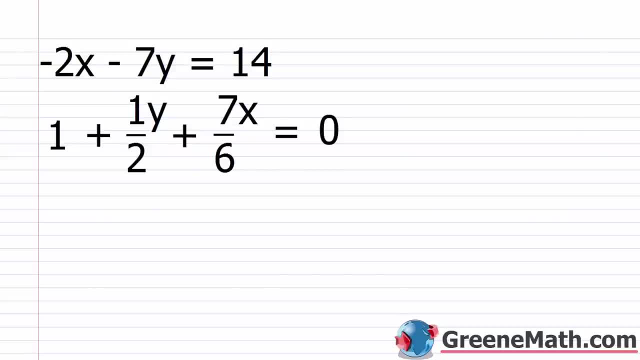 All right, let's take a look at one final problem. Again, as you practice this, it becomes very, very easy. 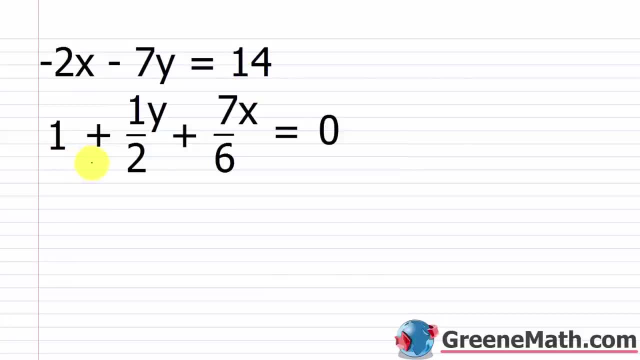 We have negative 2x minus 7y equals 14, and we have 1 plus 1 half y plus 7, 6x equals 0. 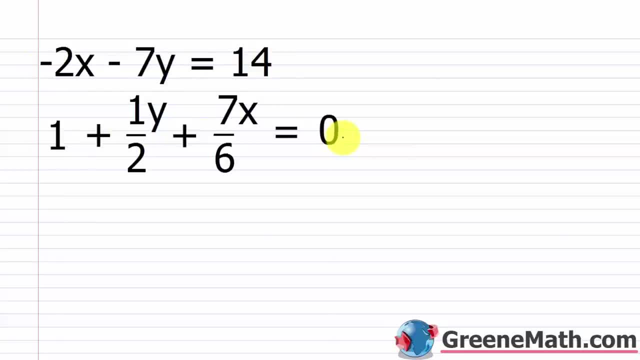 So this equation is in standard form. This one's not. 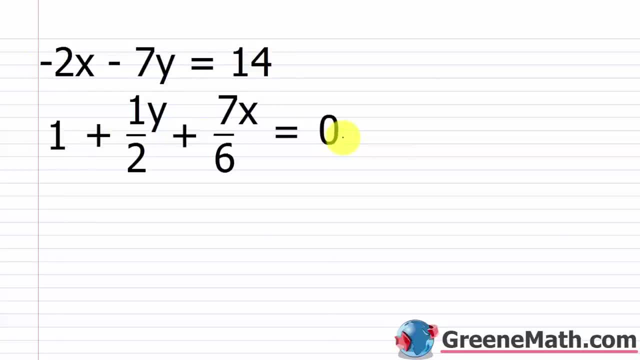 instead of negative 2, it's negative 2, so it's negative 2, plus 7, 6x equals 0.. Standard form. this one's not, So let's go ahead and fix that. So, because this is all addition. 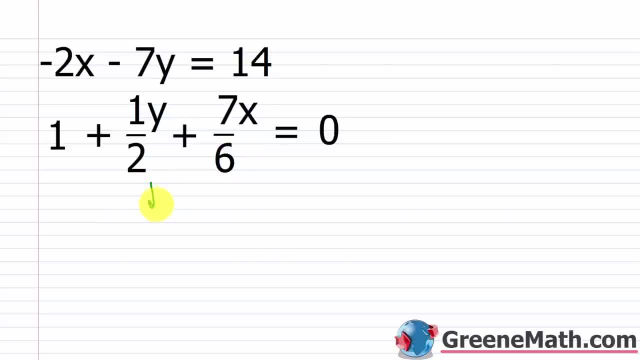 here I can switch the order around. I could rewrite this as 7, 6x plus 1, half y plus 1 equals 0. And I could simply subtract 1 away from each side of the equation And I would just. 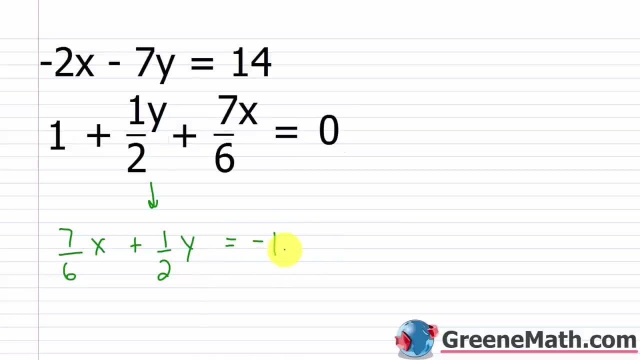 basically have equals negative 1. Now, a lot of us don't like to work with fractions, So it's very easy to clear fractions from an equation. So I'm going to go ahead and do that. So I'm going to go ahead and do that. So let's go ahead and do that. So I'm going to go ahead and do that, So. 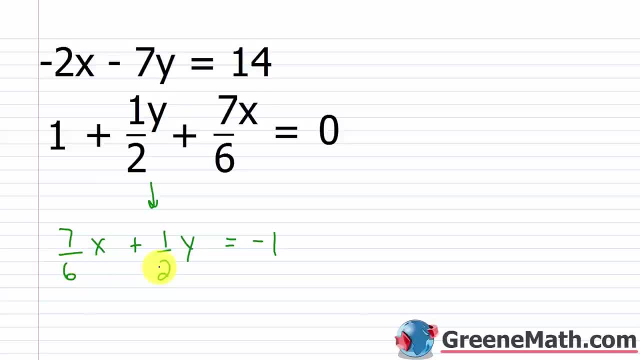 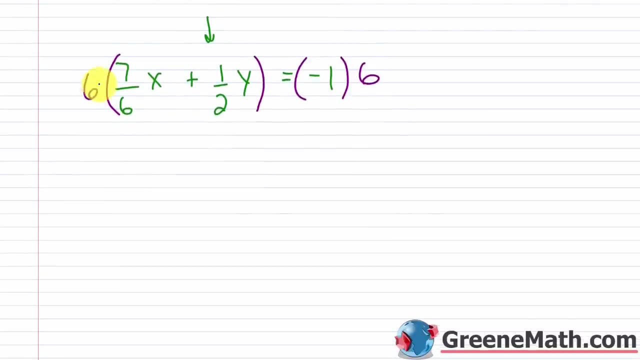 you multiply both sides by the LCD, The LCD here would be 6.. Let me kind of scooch this over a little bit And scroll down: So 6 times 7,, 6, the 6s would cancel. I'd have 7x. And then, when I 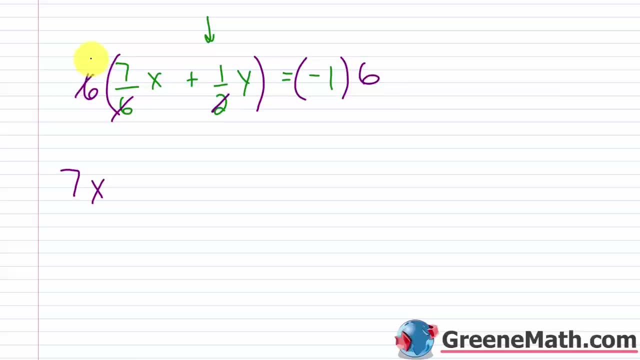 multiply 6 times 1, half the 6 would cancel with the 2 and give me a 3.. 3 times 1 is 3.. So I'd have plus 3y And this is equal to negative 1 times 6 or negative 6.. So I have 7x plus 3y. 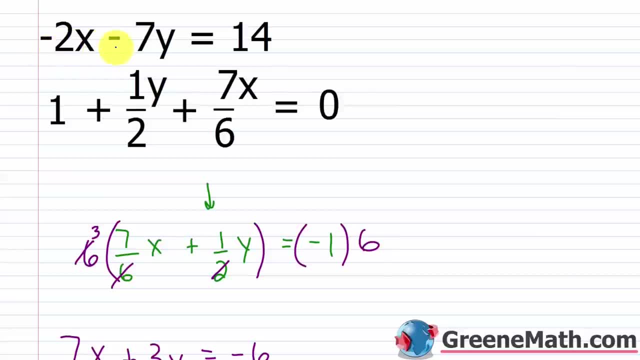 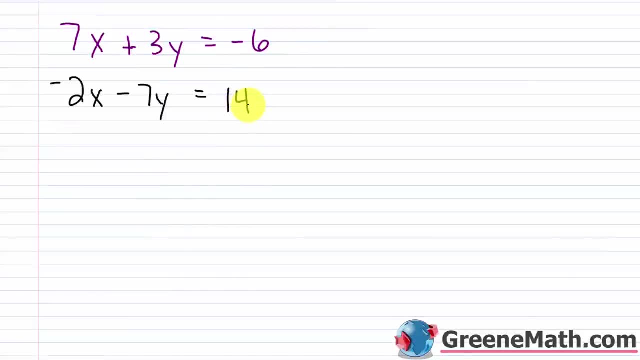 equals negative 6.. And then my other equation again is negative: 2x minus 7y equals 14.. All right, so now that I have my two equations in standard form, again I want to check and see: do I have any coefficients for any of the variables that are? 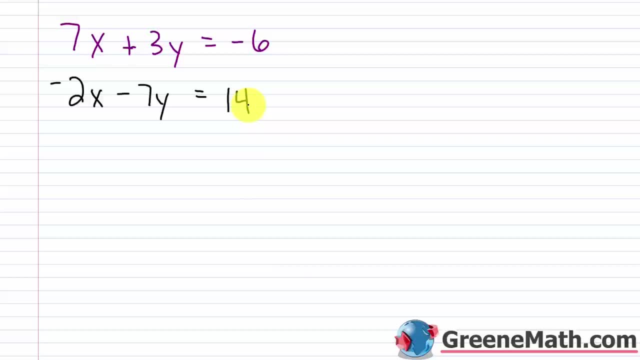 opposites. So, in other words, I look at the x variable, in each case I have a 7 and a negative 2. So it's a no-go there. I look at the y variable: I have a 3 and a negative 7. Doesn't work there. 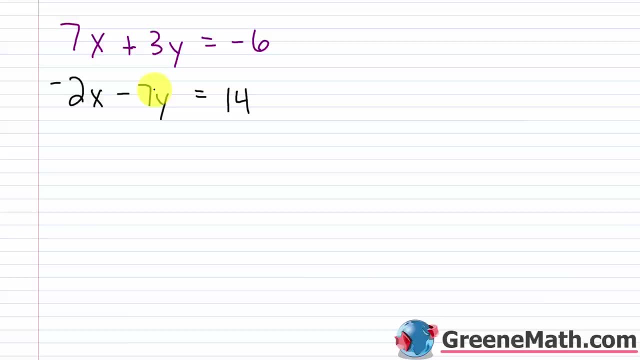 either. So now I've got to do an additional step. I've got to transform one or both equations into equivalent equations, where the coefficients for one pair of variable terms are going to be opposites. right, That's crucial to the elimination method. So let's just work with x. I see that one. 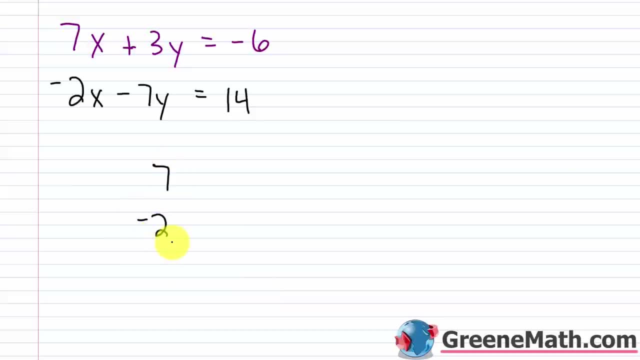 coefficient is 7.. The other is negative 2.. So I just like to write them out there. Think about: okay. well, if I multiply 7 by 2, I'd get 14.. If I multiply negative 2 by 7, I get negative 14.. 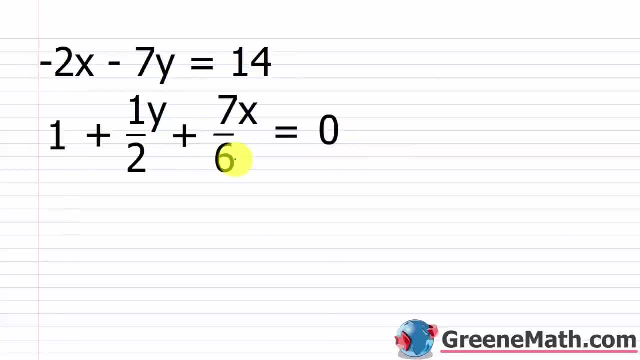 So let's go ahead and fix that. So because this is all addition here, I can switch the order around. 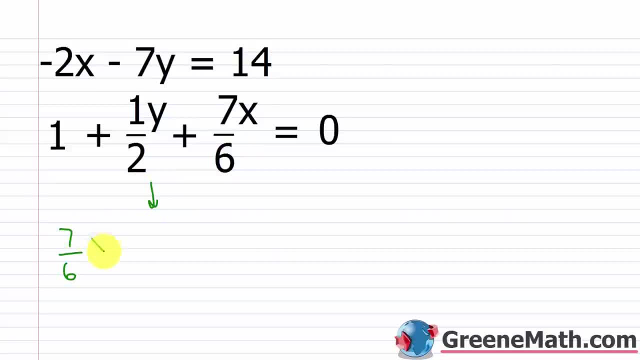 I could rewrite this as 7, 6x plus 1 half y plus 1 equals 0, and I could simply subtract 1 away from each side of the equation, and I would just basically have equals negative 1. 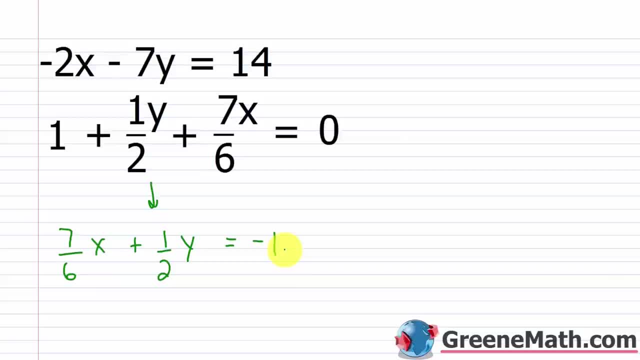 Now, a lot of us don't like to work with fractions, so it's very easy to clear fractions from an equation. 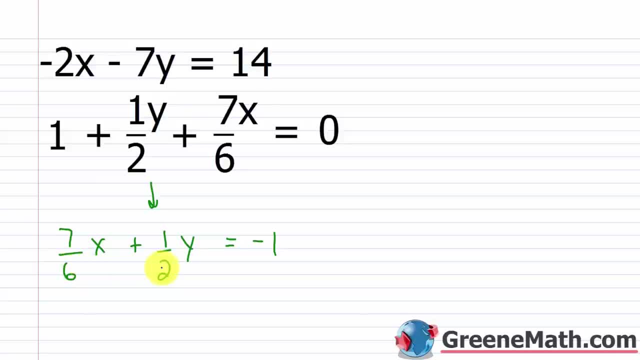 You multiply both sides by the LCD. You multiply both sides by the LCD. You multiply both sides by the LCD. The LCD here would be 6. 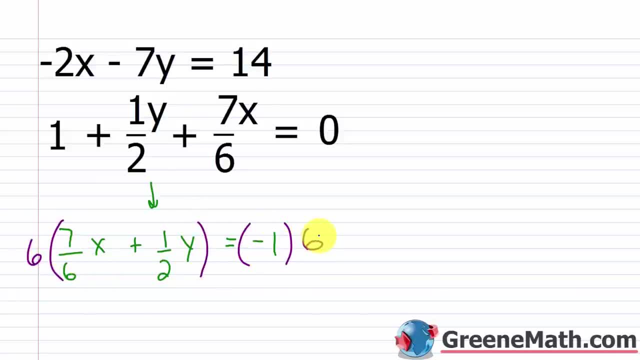 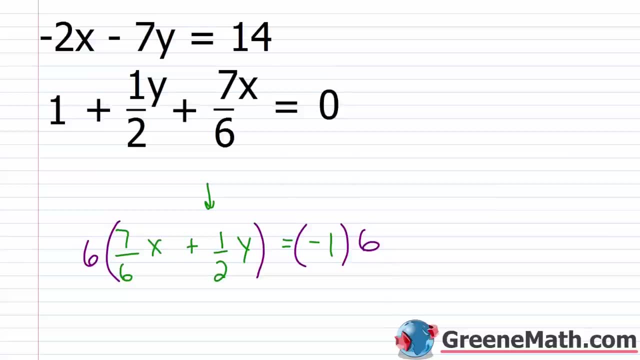 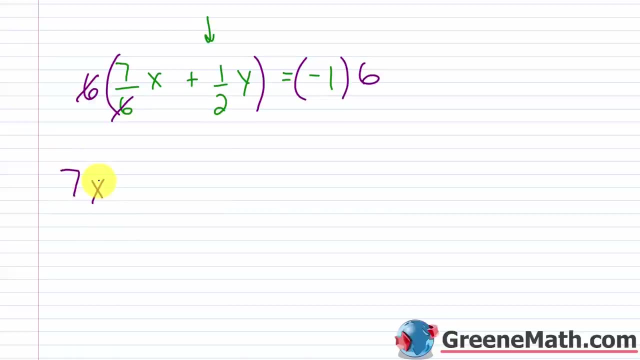 Let me kind of scooch this over a little bit and scroll down. So 6 times 7, 6, the 6's would cancel. I'd have 7x, and then when I multiply 6 times 1 half, the 6 would cancel with the 2 and give me a 3. 3 times 1 is 3, so I'd have plus 3y. And this is equal to 3y. So I'd have plus 3y. All right. 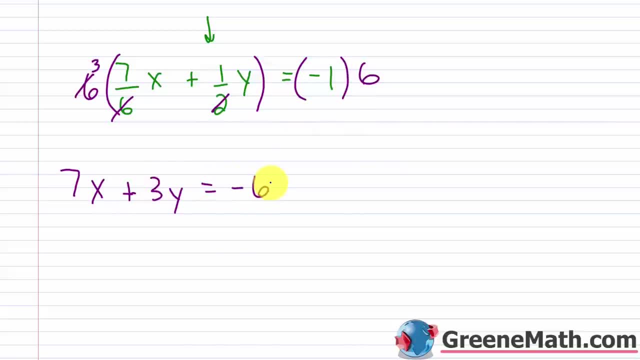 So I'm going to do negative 1 times 6, or negative 6. So I have 7x plus 3y equals negative 6. 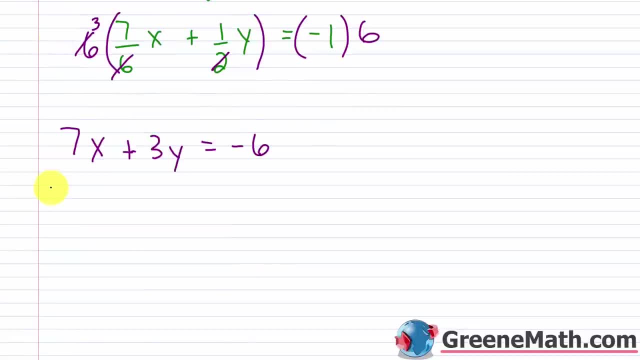 And then my other equation again is negative 2x minus 7y equals 14. All right. 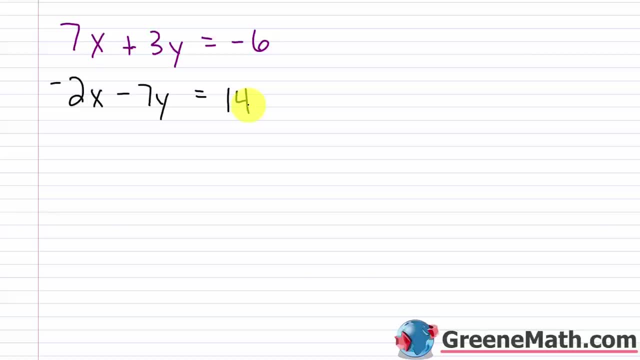 So now that I have my two equations in standard form, again, I want to check and see, do I have any coefficients for any of the variables that are opposites? So in other words, I look at the x variable in each case. I have a 7 and a negative 2. So it's a no-go there. 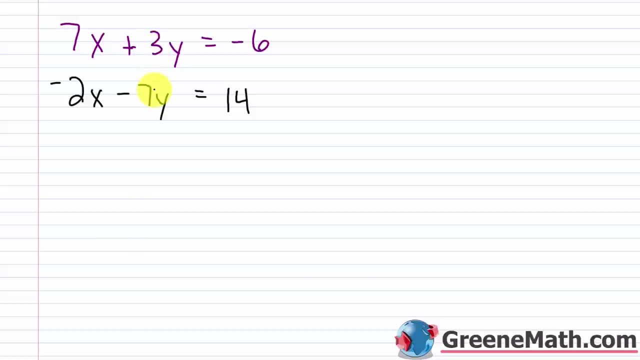 I look at the y variable. I have a 3 and a negative 7. Doesn't work there either. 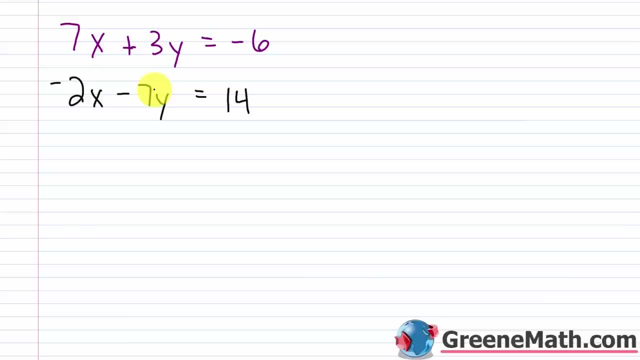 So now I've got to do an additional step. I've got to transform one or both equations into equivalent equations where the coefficients for one pair of variable terms are going to be opposites. All right. 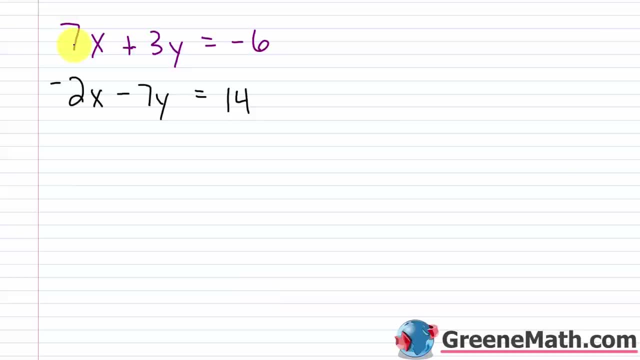 That's crucial to the elimination method. So let's just work with x. I see that one coefficient is 7. The other is negative 2. So I just like to write them out there. Think about it. Okay. So if I multiply negative 2 by 2, I'd get 14. If I multiply negative 2 by 7, I get negative 14. 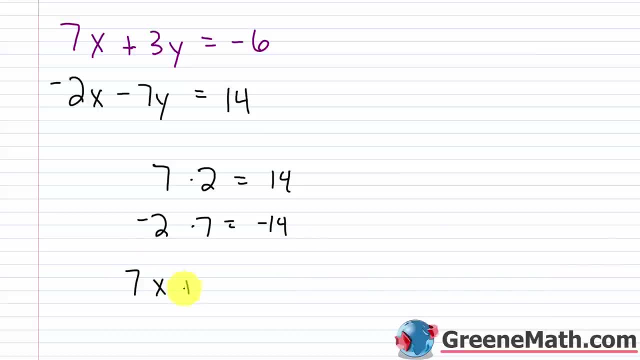 So I'm going to multiply my top equation by 2, so 7x plus 3y equals negative 6. 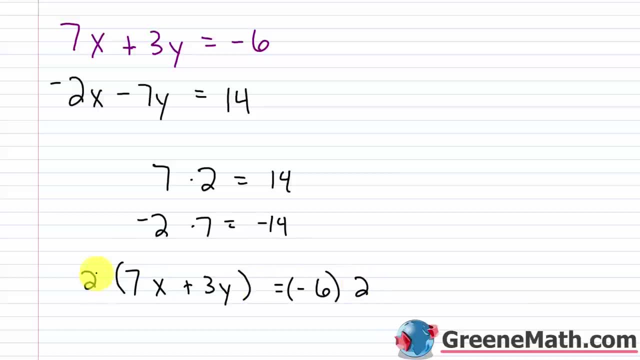 Again, I'm just going to multiply this by 2, and I'm going to multiply my bottom equation by 7. 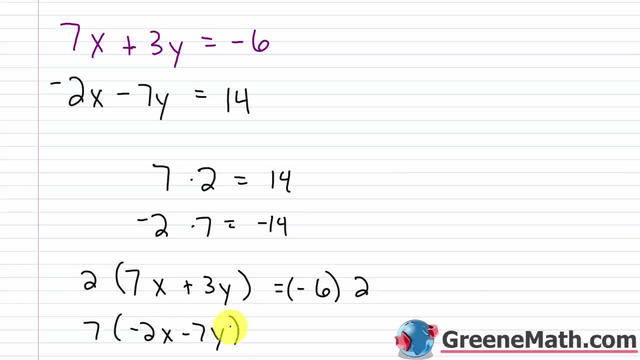 So we're going to have negative 2x minus 7y. That's multiplied by 7. This equals. We have 14. That's multiplied by 7. So 2 times 7x is 7. 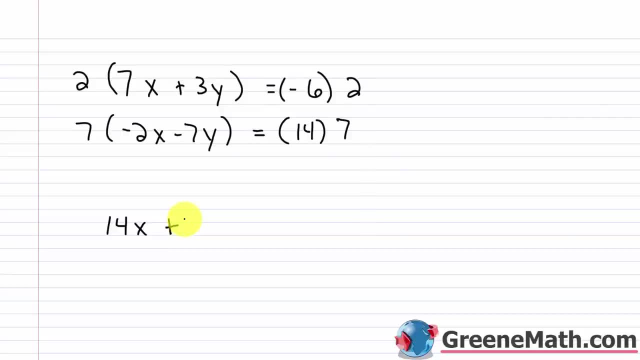 That's 14x plus 2 times 3y. That's 6y. 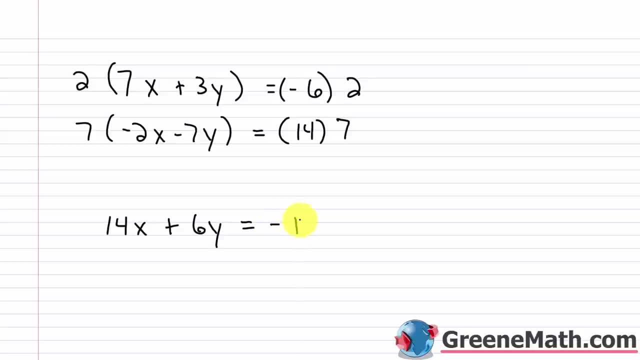 And this equals negative 6 times 2. That's negative 12. Over here, I have 7 times negative 2x. That's negative 14x. 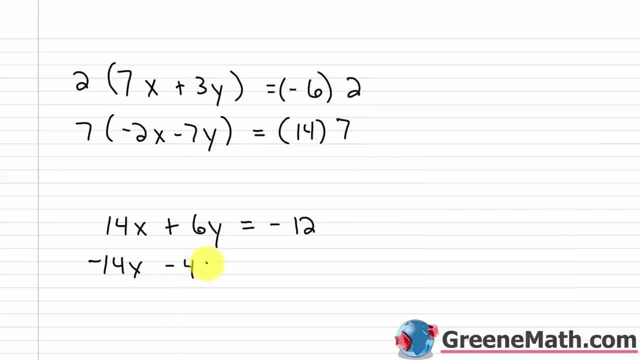 7 times negative 7y is negative 49y. This equals 7 times 14, which is 98. 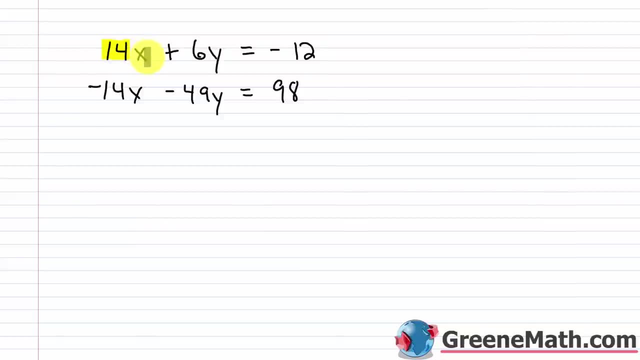 So now we can see that we have a 14. 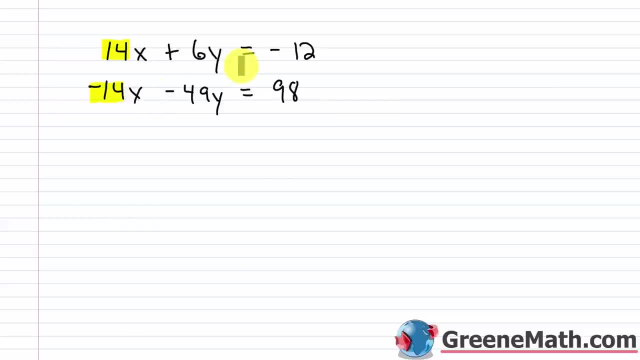 That's the coefficient for x there and a negative 14. That's the coefficient for x there. 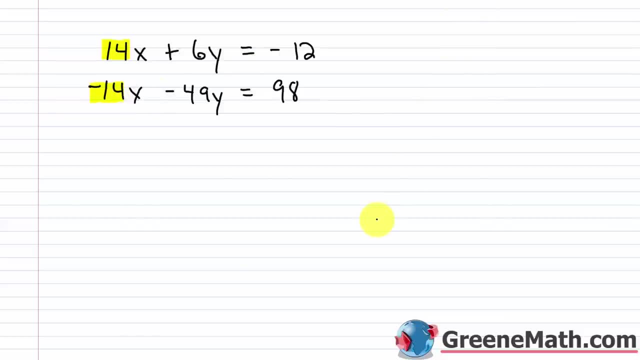 So we've successfully transformed these two equations such that one variable is going to be eliminated when we do our next step. So in the next step, remember, we add the two left sides together, set that equal to the sum of the two right sides. So 14x plus negative 14x would be 0. This is eliminated. 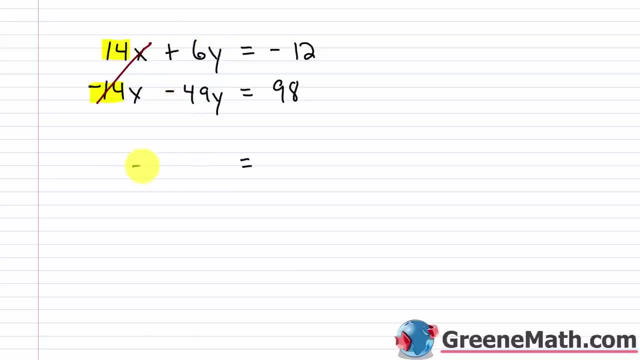 And then 6y plus negative 49y is negative 43y. Over here, negative 12 plus 98. 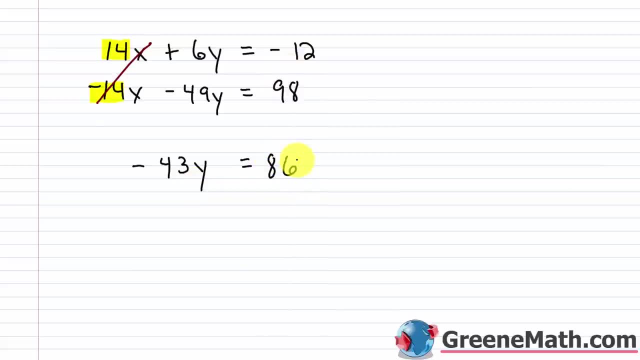 That's going to be 86. 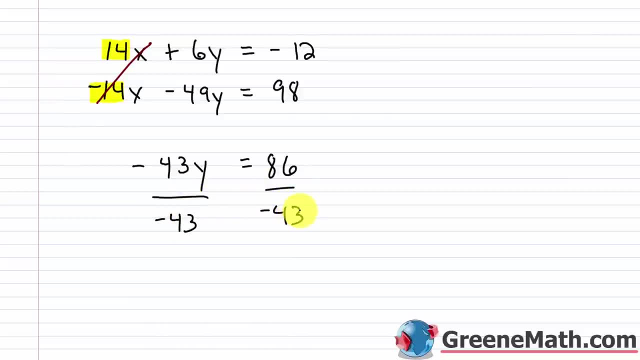 Divide both sides of the equation by negative 43. To isolate y, you're going to get that y is equal to negative 2. Again, y equals negative 2. 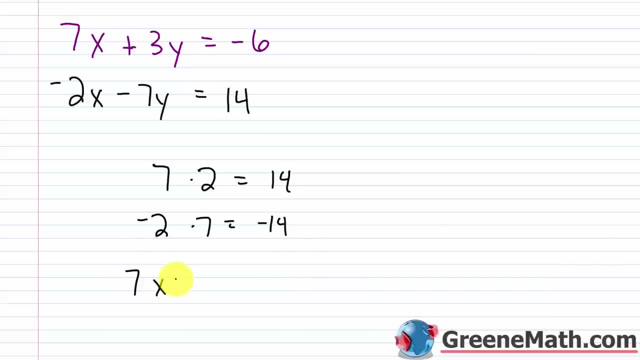 So I'm going to multiply my top equation by 2.. So 7x plus 3y equals negative 6.. Again, I'm just going to multiply this by 2.. I'm going to multiply my bottom equation by 7.. So we're. 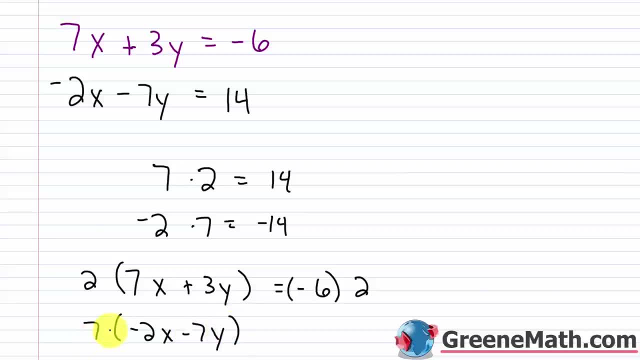 going to have negative 2x minus 7y. That's my bottom equation. So I'm going to multiply my top equation by 7. This equals we have 14.. That's multiplied by 7.. So 2 times 7x is 14x. 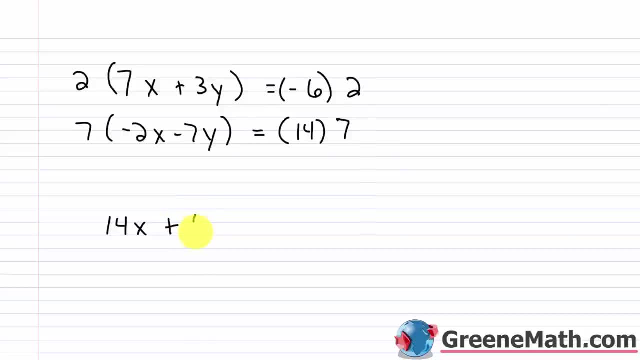 plus 2 times 3y, That's 6y, And this equals negative 6 times 2.. That's negative 12.. Over here I have 7 times negative: 2x. That's negative. 14x. 7 times negative: 7y is negative. 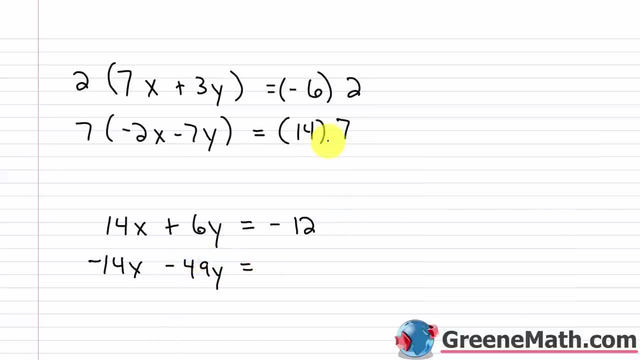 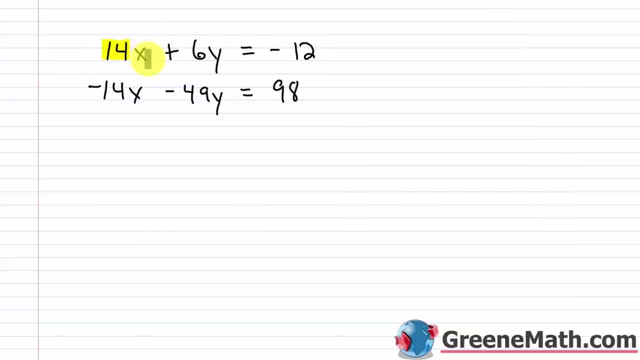 49y. This equals 7 times 14, which is 98. So now we can see that we have a 14- that's the coefficient for x there- and a negative 14- that's the coefficient for x there. So we have successfully transformed these two equations such that one variable is going to: 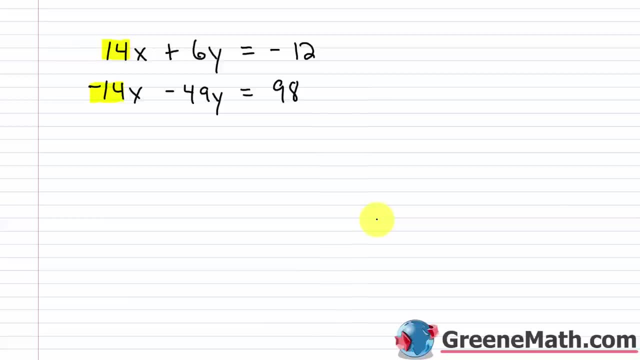 be eliminated when we do our next step. So in the next step, remember, we add the two left sides together. set that equal to the sum of the two right sides. So 14x plus negative 14x would be zero. This is eliminated. And then 6y plus negative 49y is negative 43y. So we have a 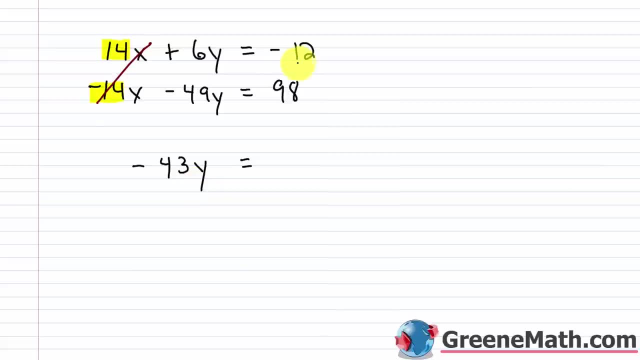 3y Over here. negative 12 plus 98 is going to be 86. Divide both sides of the equation by negative 43 to isolate y And you're going to get that y is equal to negative 2.. Again, y equals negative 2.. 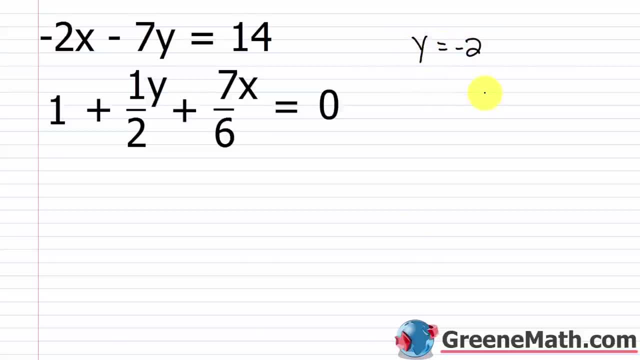 And now I can plug this back in for y in either original equation. I'm going to go ahead and use this one because it actually looks like it's easier. So we'd have 1 plus 1, half times negative. 2 plus 7, 6x equals 0. So this would cancel and be negative 1.. So you'd have 1 plus negative 1.. 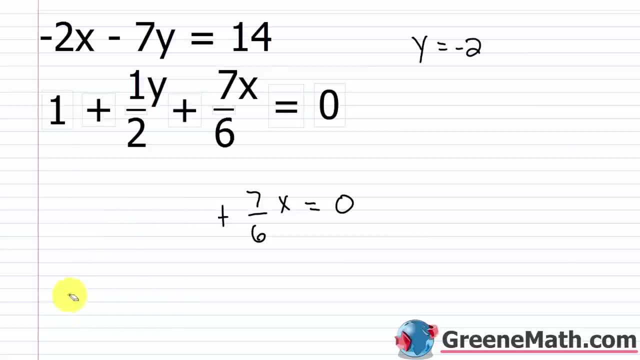 That's 0. So this whole thing is just gone. So basically I have 7: 6x equals 0. We know that can only be true if x is 0. So I know x is 0 here And again. now we just want to check the ordered pair: 0 comma negative 2.. And each original: 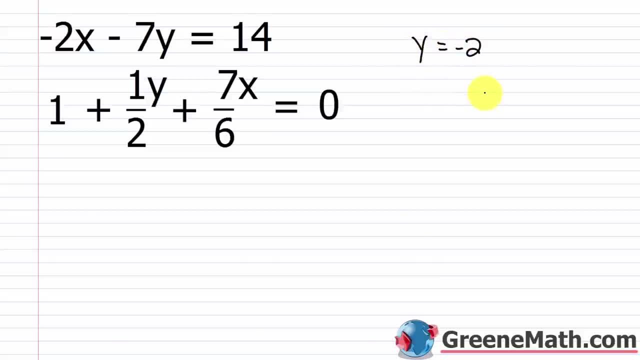 Now I can plug this back in for y in either original equation. I'm going to go ahead and use this one because it actually looks like it's easier. So we'd have 1 plus 1 half times negative 2 plus 7 6x equals 0. So this would cancel and be negative 1. 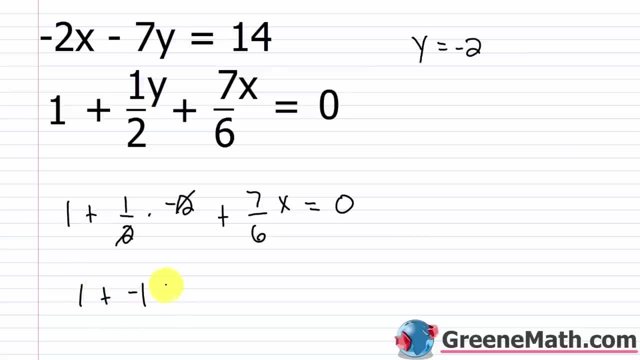 So you'd have 1 plus negative 1. That's 0. 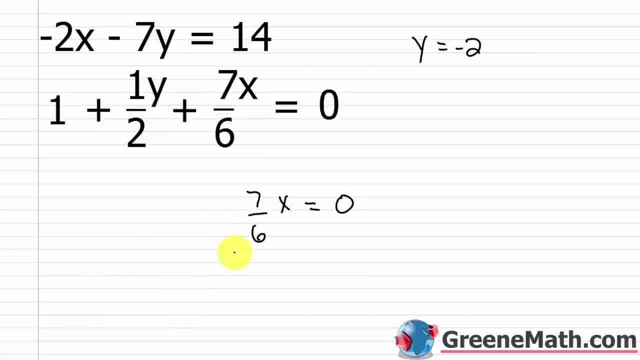 So this whole thing is just gone. So basically I have 7 6x equals 0. 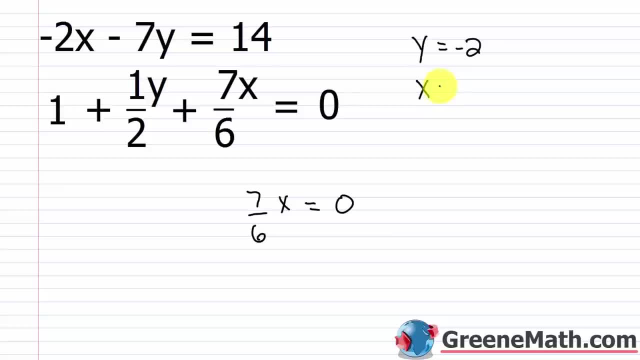 We know that can only be true if x is 0. So I know x is 0 here. 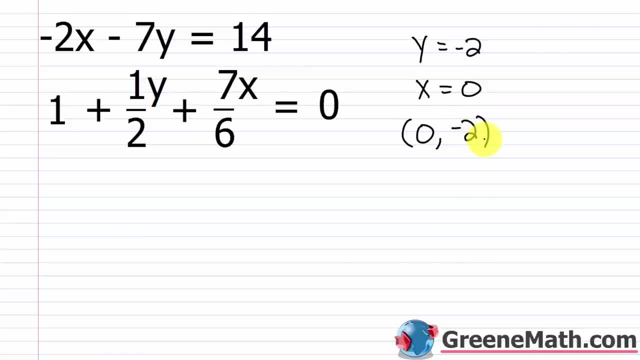 And again, now we just want to check the ordered pair 0, negative 2 in each original equation. Make sure that it's a solution for the system. So I would have... Okay. 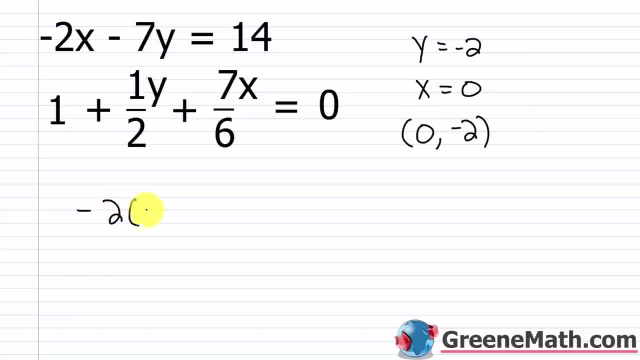 So we have negative 2 times x, we have a 0 for x, minus 7 times y, we have a negative 2 for y, equals 14. This is going to go away. 0 times anything is just 0. I have negative 7 times negative 2. That's going to give me 14. So I get 14 equals 14. 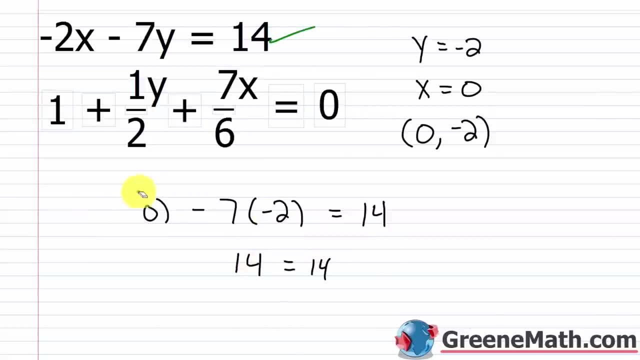 So it does check out here. In the second one, I have 1 plus 1 half times negative 2 plus 7 6 times 0 equals 0. We know this is going to go away because 0 times anything is just 0. And I know this is going to cancel with this and become negative 1. So essentially what I'm going to have is 1 plus negative 1, which is 0. So I get 0 equals 0. So it checks out here as well. 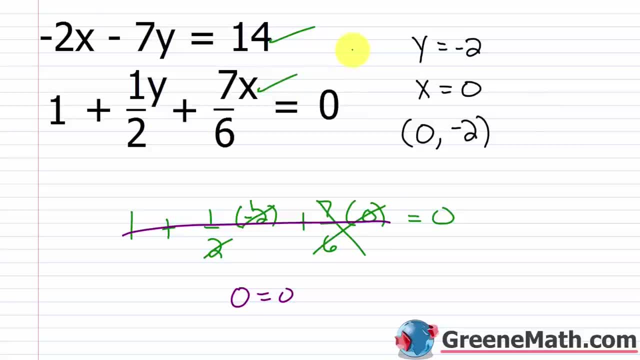 So 0 comma negative 2, that ordered pair, is a solution for the system. 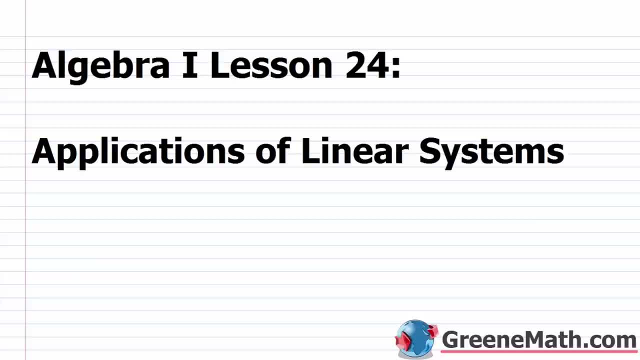 Hello and welcome to Algebra 1 Lesson 24. 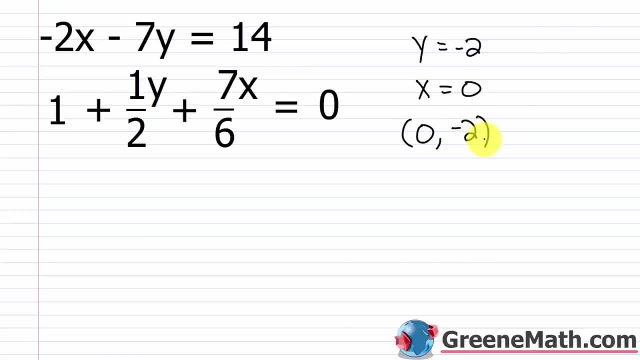 equation. make sure that it's a solution for the system. So I would have negative 2 times x. We have a 0 for x minus 7 times y. We have a negative 2 for y equals 14.. This is going to go away. 0. 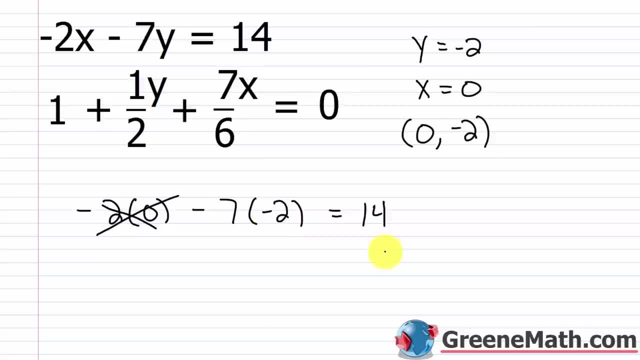 times anything is just 0.. I have negative 7 times negative 2. That's going to give me 14.. So I get 14 equals 14.. So it does check out here. And the second one: I have 1 plus 1 half times negative 2.. 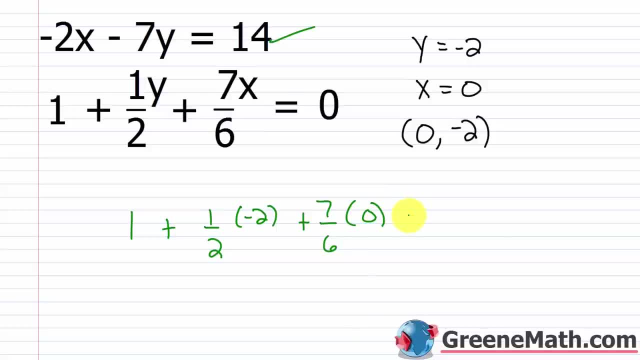 Plus 7, 6 times 0 equals 0.. We know this is going to go away, because 0 times anything is just 0. And I know this is going to cancel with this and become negative 1.. So essentially what I'm going. 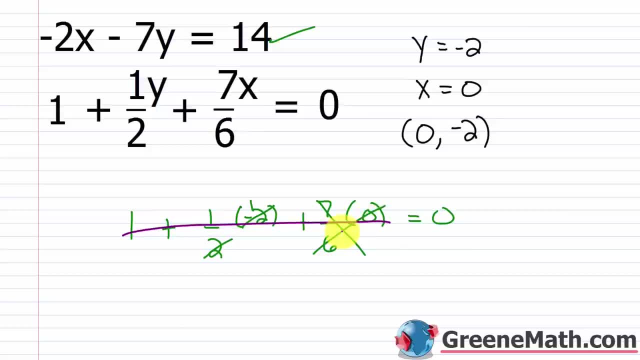 to have is 1 plus negative 1, which is 0. So I get 0 equals 0. So it checks out here as well. So 0 comma negative 2, that ordered pair is a solution for the system. 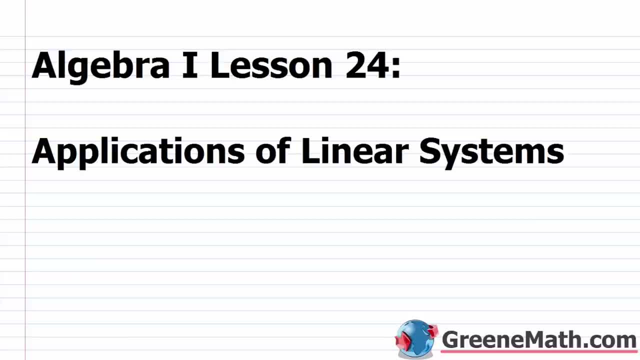 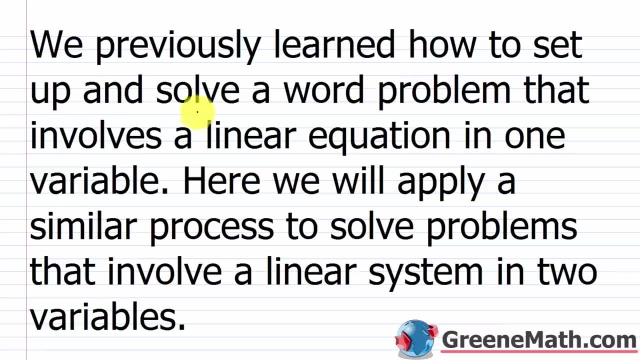 Hello and welcome to Algebra 1, Lesson 24.. In this video we're going to learn about applications of a linear system. So we previously learned how to set up and solve a word problem that involves a linear equation in one variable. Here we will apply a similar process to solve problems that involve a linear system. 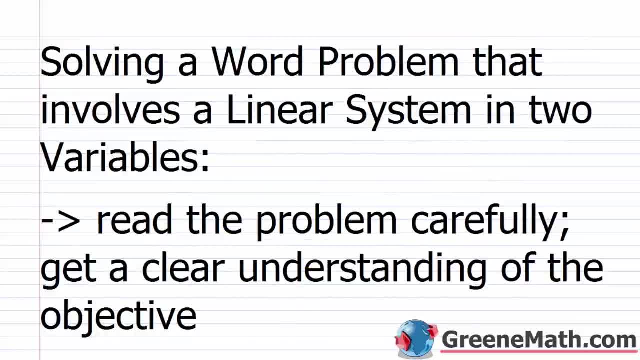 into variables. All right, so let's quickly cover this procedure- And it's just a modified version of the original one I gave you. So solving a word problem that involves a linear system into variables. thing you want to do is read the problem carefully, get a clear understanding of the objective. then 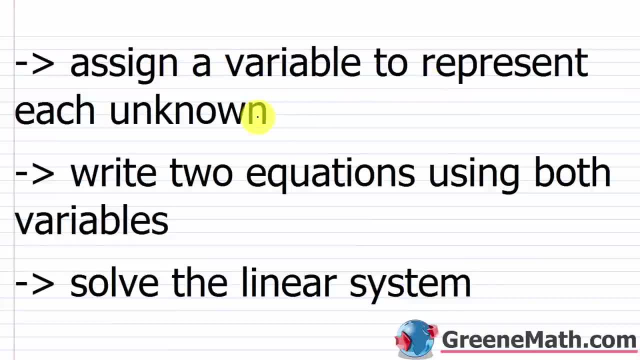 we want to assign a variable to represent each unknown and because we're working with linear systems in two variables, we're going to write two equations using both variables. then we want to solve the linear system. we're going to state the answer and, generally speaking, when we're working, 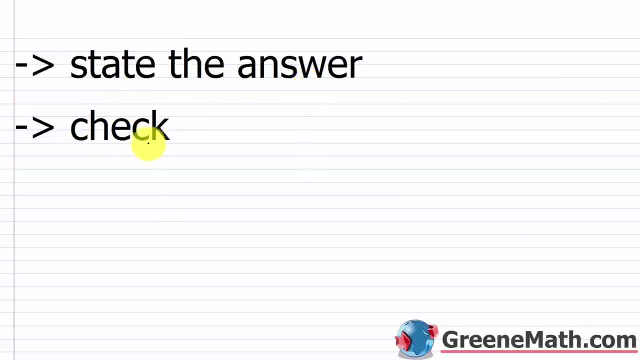 with word problems, we want to make a nice little sentence and then, lastly, we're going to check and remember. with word problems, we want to make sure that the answer is reasonable. if you had a question like how many cars were produced at a factory and you get negative 37.2, it's probably not the right. 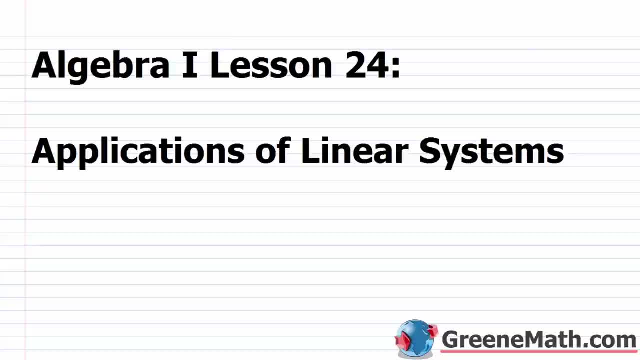 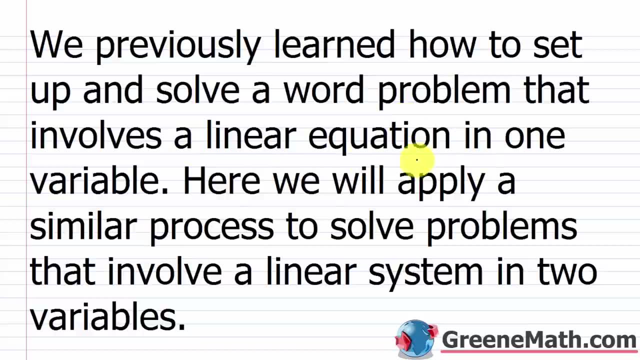 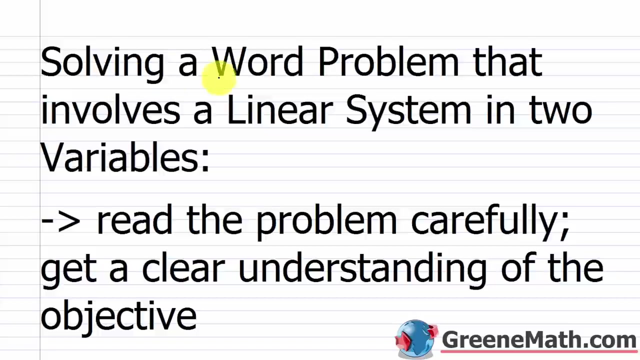 In this video, we're going to learn about applications of a linear system. So we previously learned how to set up and solve a word problem that involves a linear equation in one variable. Here we will apply a similar process to solve problems that involve a linear system in two variables. All right, so let's quickly cover this procedure, and it's just a modified version of the original one I gave you. So solving a word problem that involves a linear system in two variables. So obviously the first thing you want to do is read the problem carefully, get a clear understanding of the objective. 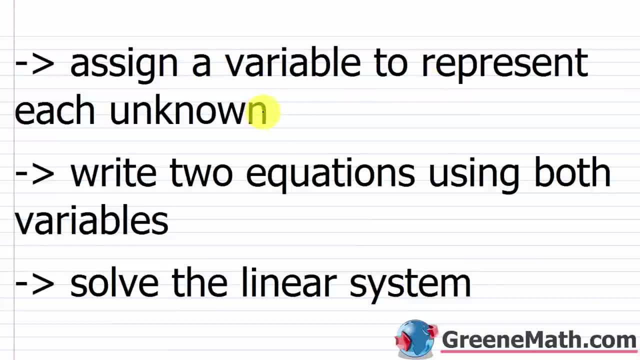 Then we want to assign a variable to represent each unknown. And because we're working with linear systems in two variables, we're going to write two equations using both variables. 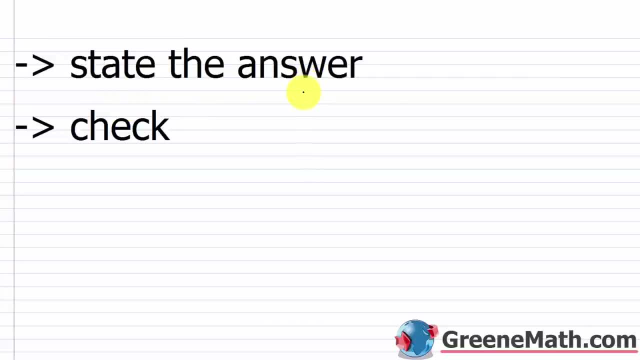 Then we want to solve the linear system. We're going to state the answer. And generally speaking when we're working with word problems, we want to make a nice little sentence. 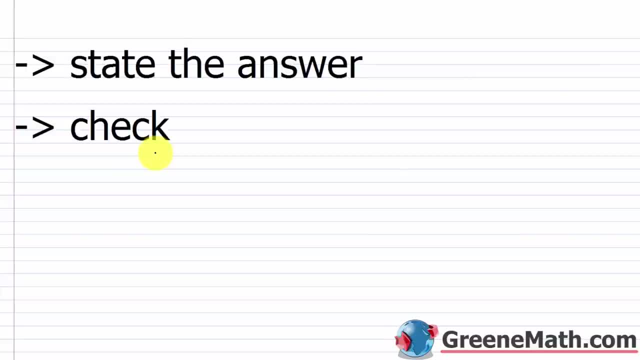 And then lastly, we're going to check. And remember with word problems, we want to make sure that the answer is reasonable. If you had a question like, how many cars were produced at a factory? And you can actually say to that answer that there are two variables. They will use two variables. So you'll have two variables as well. All right. 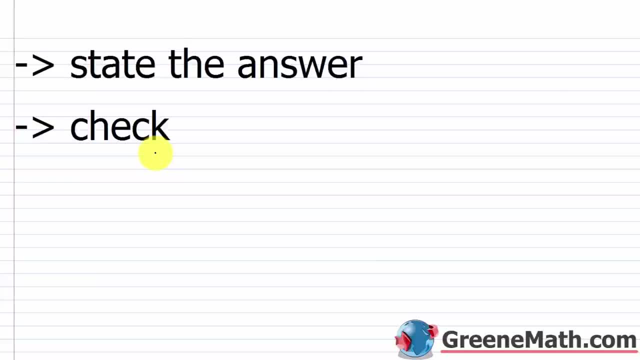 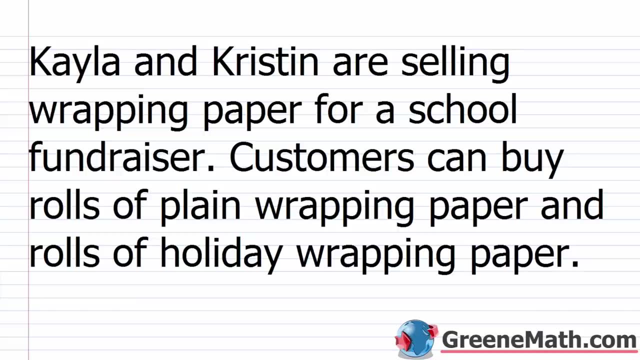 you get negative 37.2, it's probably not the right answer, right? The factor would produce either zero or some positive integer amount. All right, let's go ahead and take a look at the first problem. We have enough experience with word problems to just kind of jump right in. 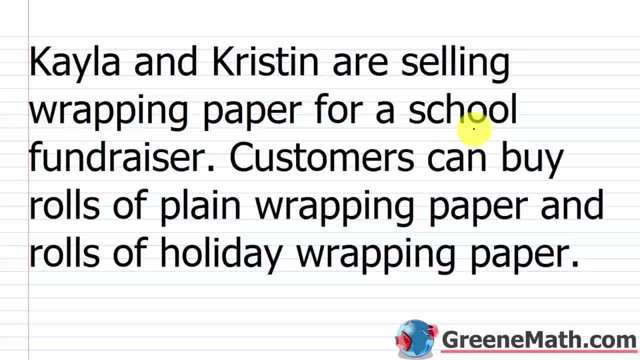 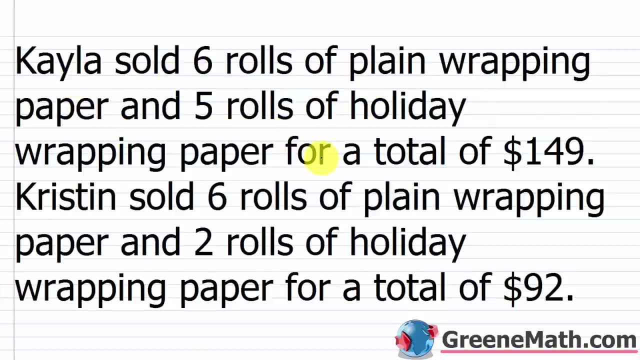 So Kayla and Kristen are selling wrapping paper for a school fundraiser. Customers can buy rolls of plain wrapping paper and rolls of holiday wrapping paper. So Kayla sold six rolls of plain wrapping paper and five rolls of holiday wrapping paper for a total of $149. 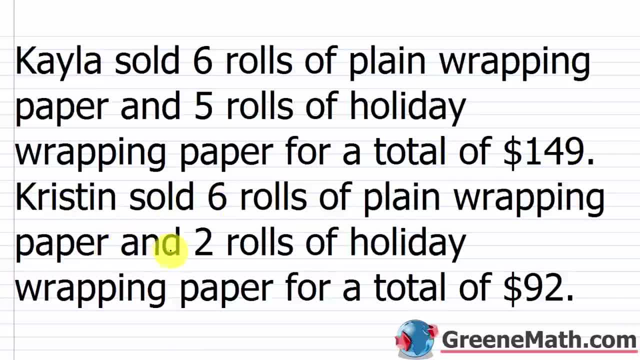 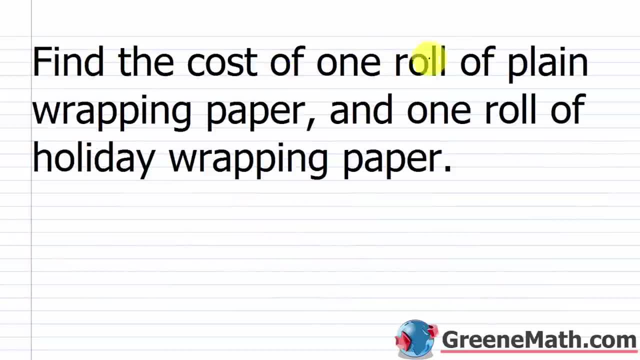 Kristen sold six rolls of plain wrapping paper and two rolls of holiday wrapping paper for a total of $92. So we want to find the cost of one roll of plain wrapping paper and one roll of 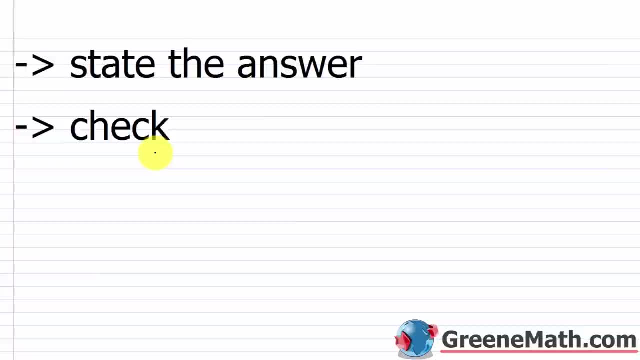 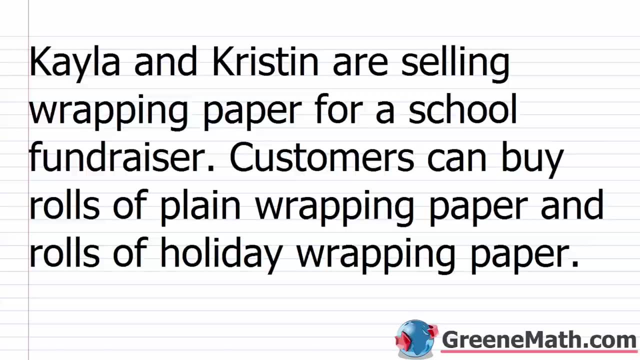 answer right, the factory would produce either zero or some positive integer amount. all right, let's go ahead and take a look at the first problem. we have enough experience with word problems to just kind of jump right in. so kayla and kristin are selling wrapping paper for a school fundraiser customers. 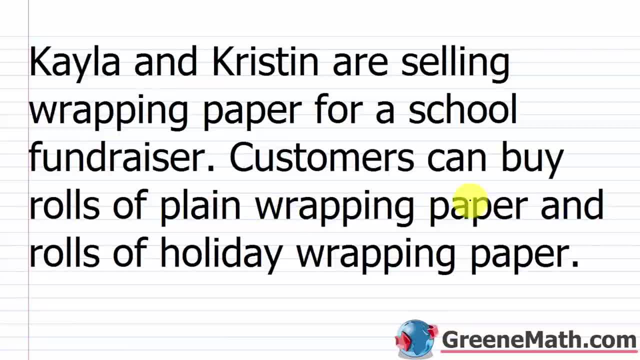 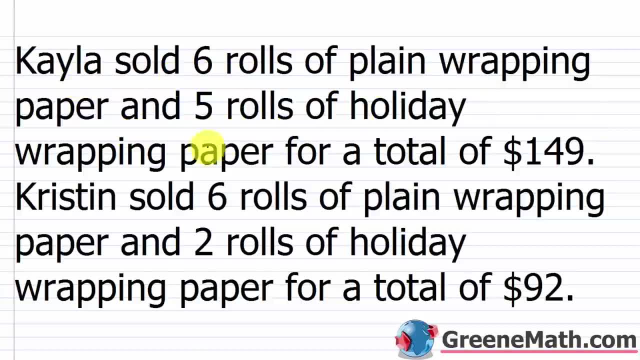 can buy rolls of plain wrapping paper and rolls of holiday wrapping paper. so kayla sold six rolls of plain wrapping paper and five rolls of holiday wrapping paper for a total of 149. kristin sold six rolls of plain wrapping paper and two rolls of holiday wrapping paper for a total of 92. so we want to. 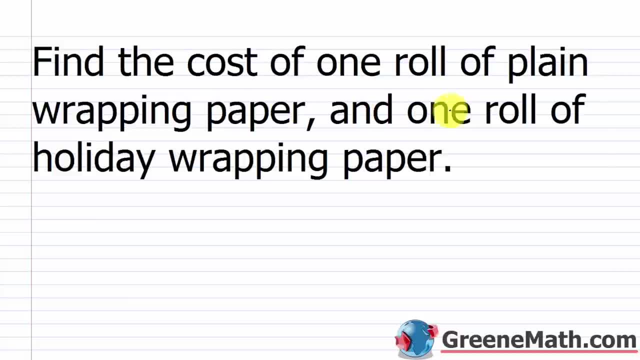 find the cost of one roll of plain wrapping paper and one roll of holiday wrapping paper. so remember, our first step was to read the problem and get a clear understanding of the objective. Well, the objective is right here: We want to find the cost of one roll of plain wrapping paper. 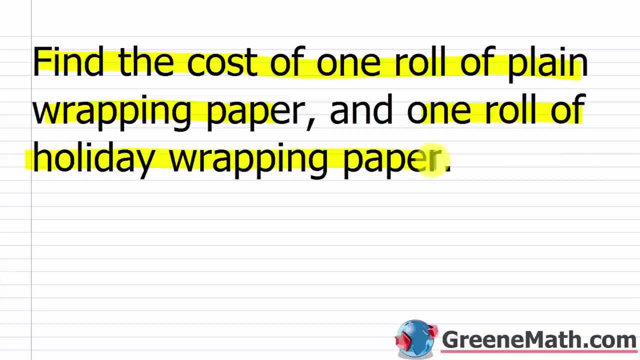 and one roll of holiday wrapping paper. So I should be able to make a nice little sentence in the end that says: the cost of one roll of plain wrapping paper is this much and the cost of one roll of holiday wrapping paper is this much. All right, so for the next step we want: 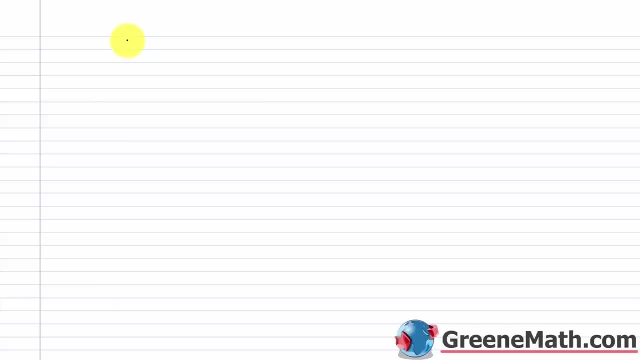 to assign a variable to represent each unknown. We don't know how much is one roll of holiday wrapping paper- I'm just going to put w period p period, as for wrapping paper. And then we also don't know how much is one roll of plain wrapping paper, So plain. 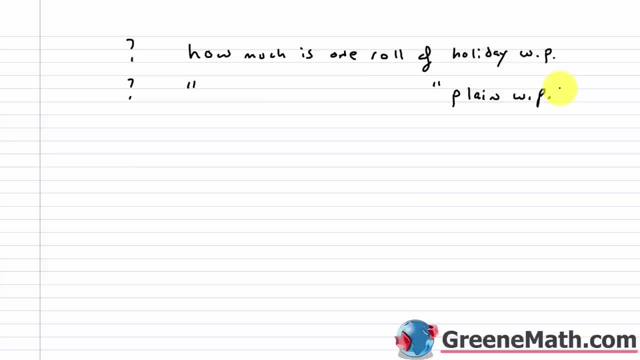 and then w period, p period, just to abbreviate a little bit. So let's assign a variable to each one And let's just use x and y, because those are the most common. So let's let x, let's let x equal the cost, Or you could say sale price. 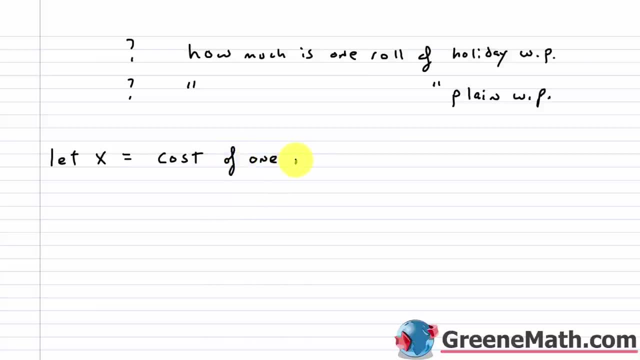 of one roll of plain wrapping paper. So I'm going to put wp for that And I'm going to put some periods there just for abbreviation: w period, p period for wrapping paper. So then, for our other unknown, I'm going to say: 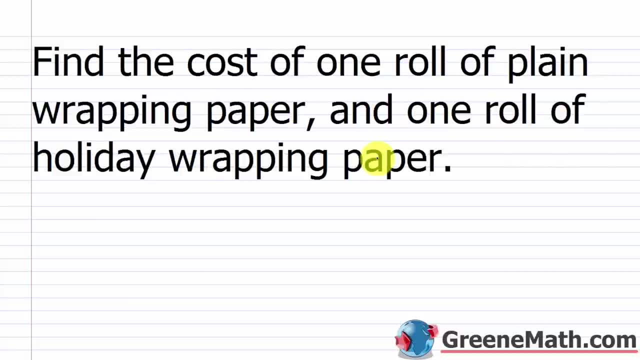 holiday wrapping paper. So remember, our first step was to read the problem and get a clear understanding of the objective. Well, the objective is right here. We want to find the cost of one roll of plain wrapping paper and one roll of holiday wrapping paper. So I should be able to make a nice little sentence in the end that says the cost of one roll of plain wrapping paper is this much and the cost of one roll of holiday wrapping paper is this much. All right, so for the next step, we want 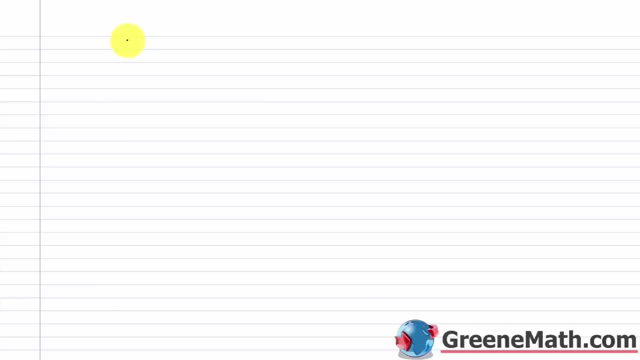 to assign a variable to represent the cost of one roll of plain wrapping paper. So we want to assign a variable to represent the cost of one roll of holiday wrapping paper. So we want to assign each unknown. We don't know how much is one roll of holiday wrapping paper. I'm just going to put W period P period as for wrapping paper. And then we also don't know how much is one roll of 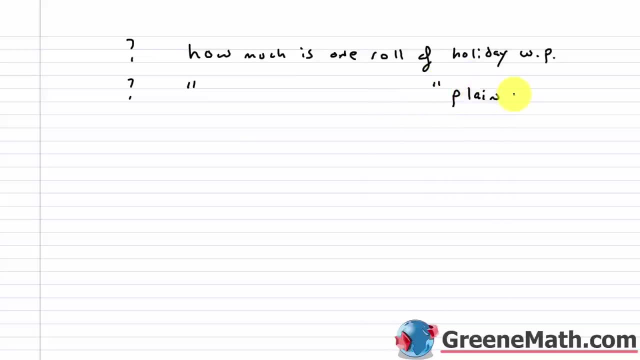 plain wrapping paper. So plain and then W period P period, just to abbreviate a little bit. So let's assign a variable. And let's just use X and Y because those are the most common. So let's let X, let's let X equal the 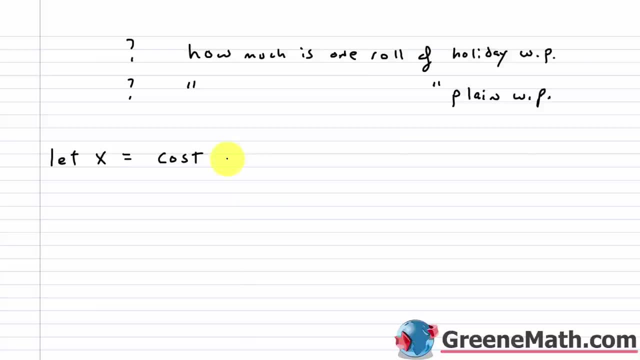 cost or you could say sale price of one roll of plain wrapping paper. So I'm going to put WP for that. And I'm going to put some periods there just for abbreviation, W period P period for wrapping 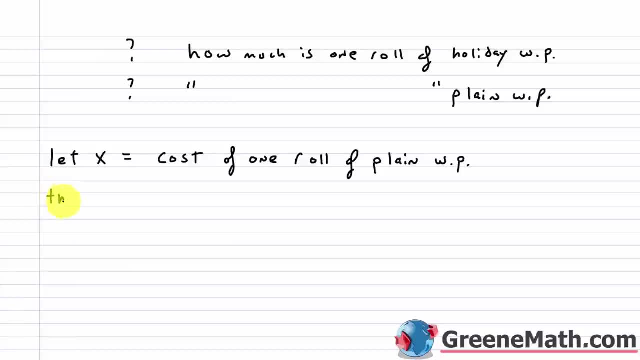 paper. So then for our other unknown, I'm going to say Y is equal to the cost of one roll of holiday wrapping paper. So again, W period P period. And don't get confused here. When I say cost, 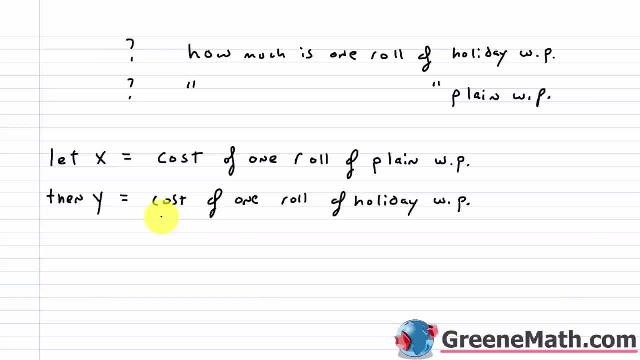 I mean sale price. So a lot of students will see that and say, well, is that the cost that they pay? And it's a little confusing. So I want to just clarify and say that the cost here when we say that we're saying the sale price, or in other words, the cost for the customer, the person who's buying it. All right, so for step three, we 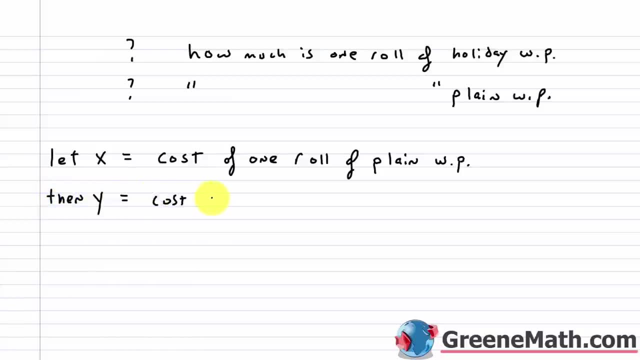 y is equal to the cost of one roll of holiday wrapping paper. So again, w period, p period. And don't get confused here: When I say cost I mean sale price. So a lot of students will see that and say they pay and it's a little confusing. So I want to just clarify and say that the cost 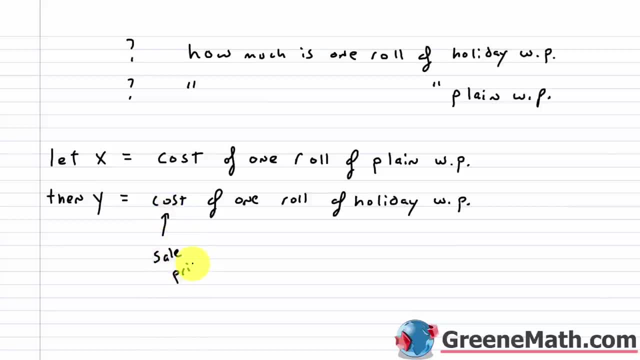 here, when we say that, we're saying the sale price, or in other words, the cost for the customer, the person who's buying it. All right, so for step three, we want to write two equations using both variables. So in order to do that, we need to read back through. 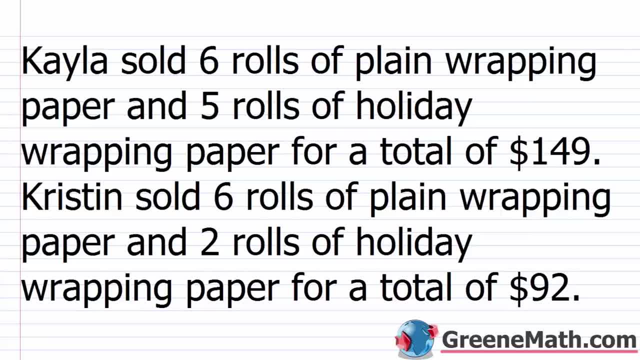 the problem. So I'm going to go to this part where all the information is given. So reading back through here, we see that Kayla sold six rolls of plain wrapping paper and five rolls of holiday wrapping paper for a total of $149.. So we can use this information to 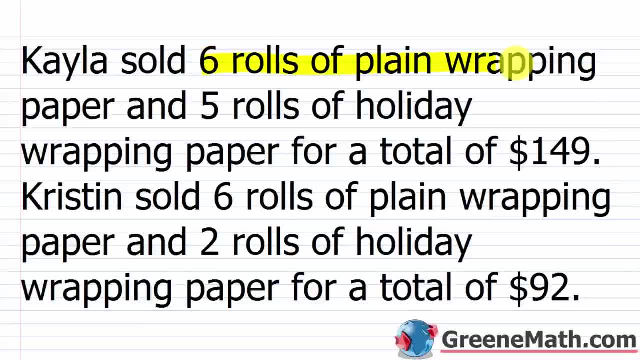 make our first equation. So six rolls of plain wrapping paper, five rolls of holiday wrapping paper, again, for a total of $149.. So putting that into an equation, just using our variables for the unknown, we would have six times x, right. x is the cost of one single roll of. 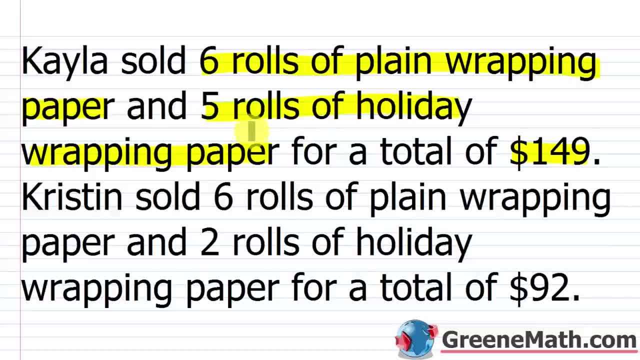 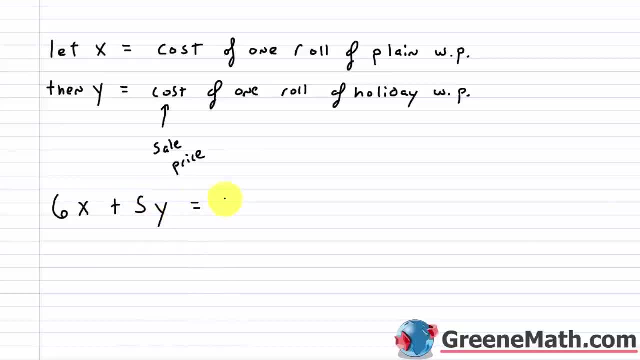 plain wrapping paper plus y. y is the cost of one roll of holiday wrapping paper- should be $149.. The total cost when these two are added together- So again this is going to be six x plus five y is equal to $149.. And let's label this so we don't get confused. So six represents the number. 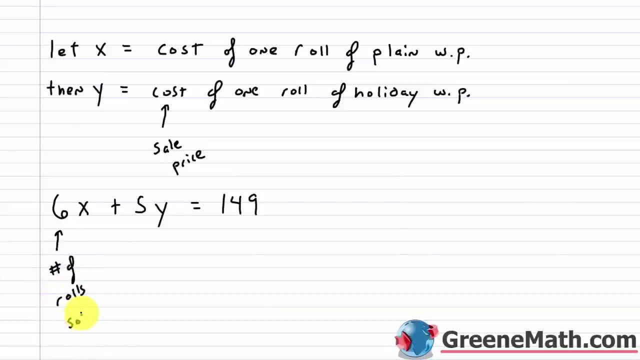 of rolls sold, And so does five. So let me draw a little arrow over to five. For example, for x, this is the cost of one roll of plain wrapping paper. So the cost of one roll of plain wrapping. let me get rid of this paper. 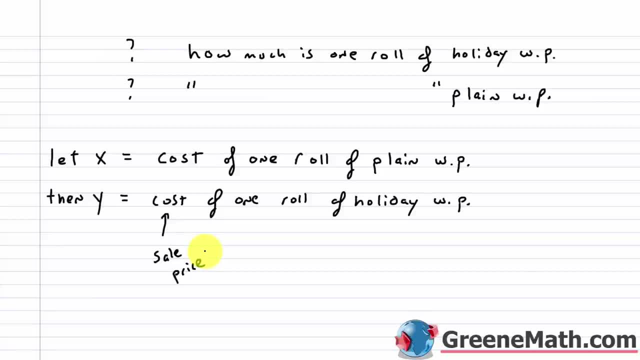 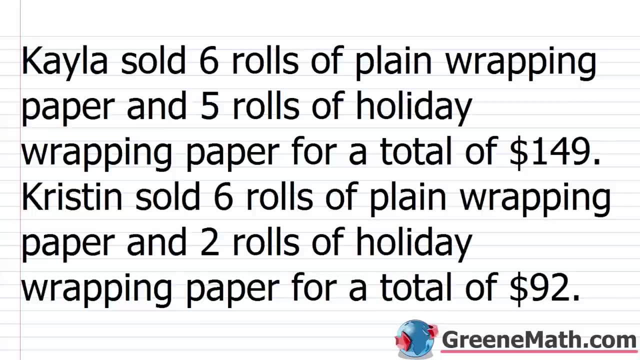 want to write two equations using both variables. So in order to do that, we need to read back through the problem. So I'm going to go to this part where all the information is given. So reading back through here, we see that Kayla sold six rolls of plain wrapping paper, and five rolls of holiday wrapping paper 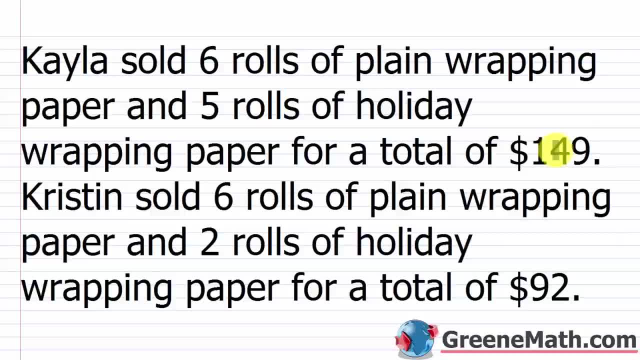 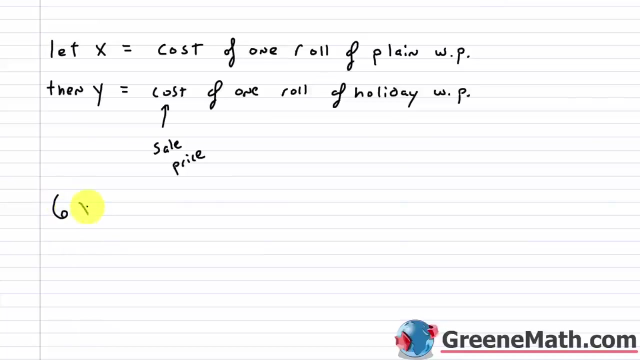 total of $149. So we can use this information to make our first equation. So six rolls of plain wrapping paper, five rolls of holiday wrapping paper, again, for a total of $149. So putting that into an equation, just using our variables for the unknown, we would have six times X, right? X is the cost of one single roll of plain wrapping paper, plus five times Y. Y is the cost of one roll of holiday wrapping paper should be $149, the total cost when these two are added together. So again, this is going to be six X plus five Y is equal to $149. And let's label this so we don't get confused. So six represents the number of rolls sold. And so does five. So let me draw a little arrow over to five. For X, this is the cost of one roll of holiday wrapping paper, plus five times Y. Y is the cost of one roll of holiday wrapping paper. So the cost of one roll of plain wrapping paper. Let me kind of get rid of this paper. Then for Y, it's the cost of one roll of holiday wrapping paper. 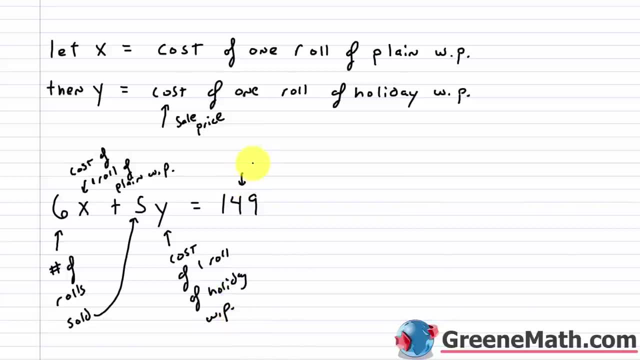 So again, $149 is the total money she brings in. So I can put the total from the sale of both. So she sells six rolls of plain wrapping paper. So that's modeled with six, the number of rolls sold, times X, which is the cost per roll, again, of plain wrapping paper. Then we add this to five, which again, is the number of rolls sold, times Y, which is the cost of one roll of holiday wrapping paper. So that's modeled with six, Y, which is the cost of one roll of holiday wrapping paper. So we sum these two amounts 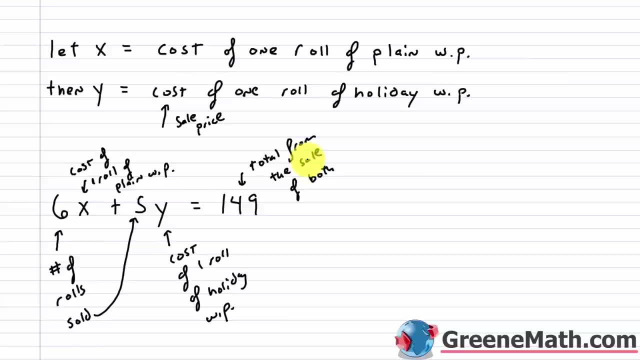 together, and we get the total amount that she gets from the sale of both. That's $149. 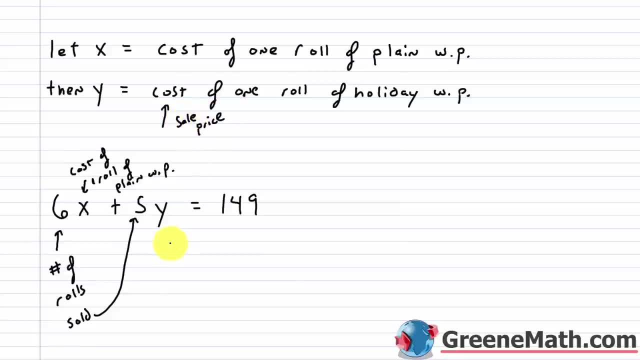 Then for y it's the cost of one roll of holiday wrapping paper: $149.. Ten collections based $149.. Then for Y it's the cost of one roll of holiday wrapping paper: $149.. Ten collections based $149, so again 149 is the total, the total money she brings in, so i can put the total from the sale. 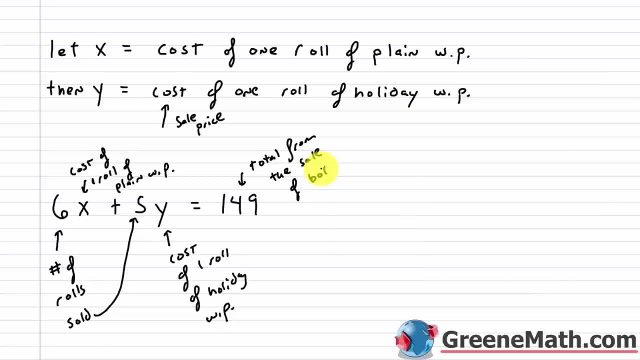 of both. so she sells six rolls of plain wrapping paper. so that's modeled with six, the number of sold times x, which is the cost per roll, again, of plain wrapping paper. then we add this to five, which again is the number of rolls sold times y, which is the cost of one roll of holiday wrapping. 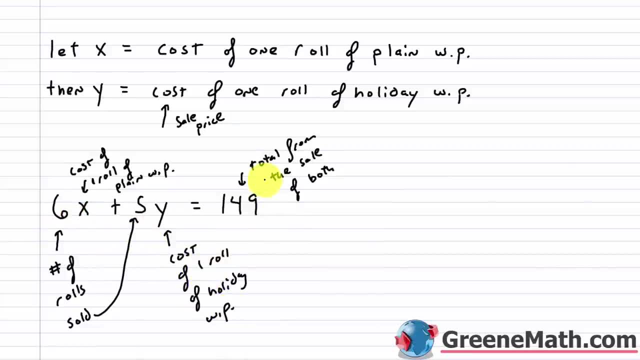 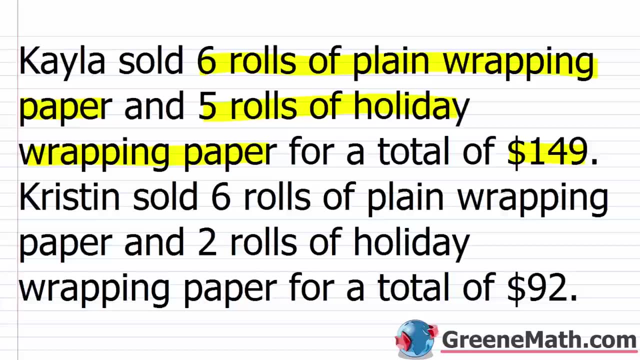 paper. so we sum these two amounts together and we get the total amount that she gets from the sale of both. that's 149. so there's your first equation. now for the second one. let's read about kristin. so kristin sold six rolls of plain wrapping paper and two rolls of holiday wrapping paper. 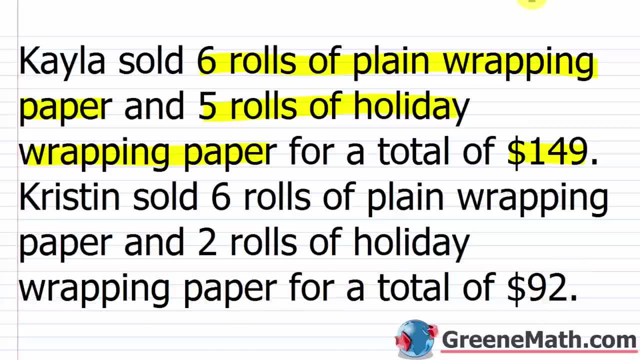 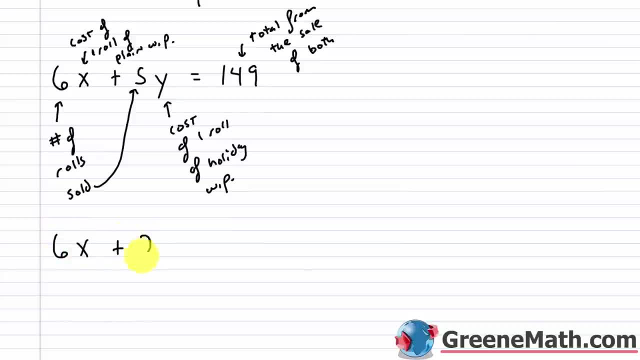 for a total of 92. i can go through and highlight that. so six rolls of plain wrapping paper, two rolls of holiday wrapping paper- again this is for 92. so we're going to come down here and just make a similar equation. so we'd have six times x plus two times y is equal to 92, and if we went, 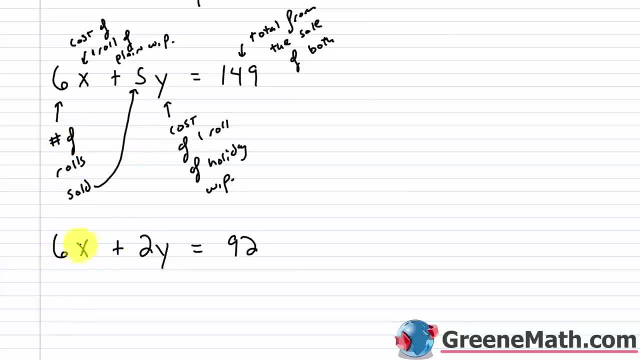 through and labeled, it would be the same right. you'd have six, which is the number of rolls sold times x, which is the cost of a single roll of plain wrapping paper plus. and then you'd have two, which again is the number of rolls sold times y, which is the cost of one roll of holiday. 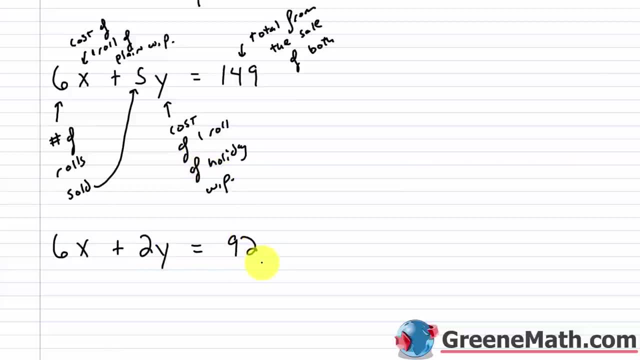 wrapping paper, and the sum here is going to equal 92, right? that's the total from the sale of both. all right, so we've correctly modeled each situation for the two girls. so let's look at these two equations now and see if we can solve this linear system. so i'm going to rewrite them. 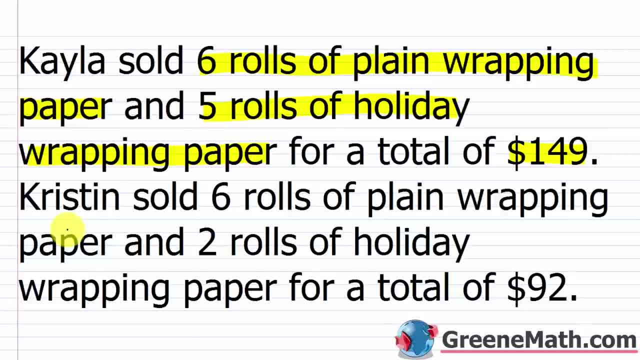 So there's your first equation. Now for the second one, let's read about Kristen. So Kristen sold six rolls of plain wrapping paper and two rolls of holiday wrapping paper for a total of $92. I can go through and highlight that. So six rolls of plain wrapping paper, two rolls of holiday wrapping paper, again, this is for $92. So we're going to come down here and just make a similar equation. 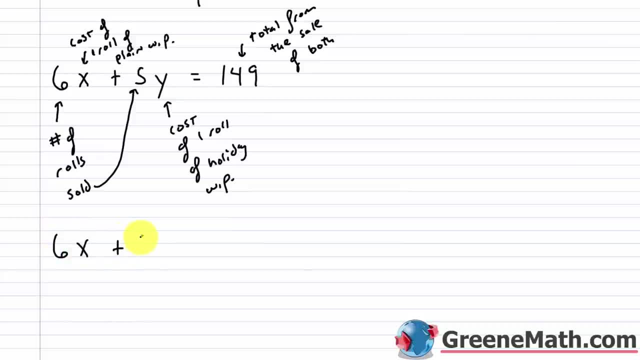 So we'd have six times X plus two times Y is equal to 92. And if we went through and labeled it, it would be the same, right? You'd have six, which is the number of rolls sold, times X, which is the cost of a single roll of plain wrapping paper, plus, and then you'd have two, which again, is the number of rolls sold, times Y, which is the cost of one roll of holiday wrapping paper. And the sum here is going to equal 92. 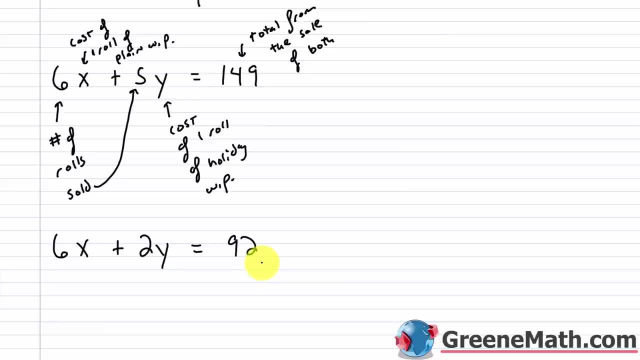 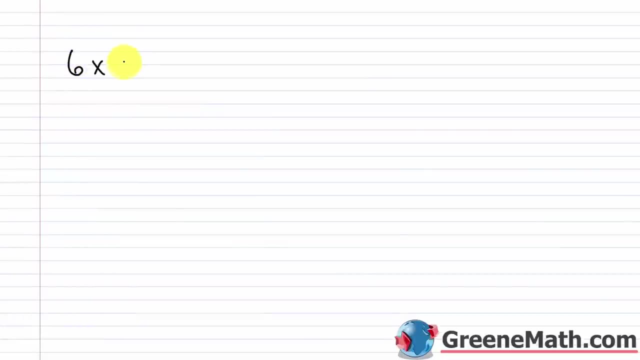 All right, that's the total from the sale of both. All right, so we've correctly modeled each situation for the two girls. So let's look at these two equations now and see if we can solve this linear system. So I'm going to rewrite them down here. So I have six X plus five Y equals 149. 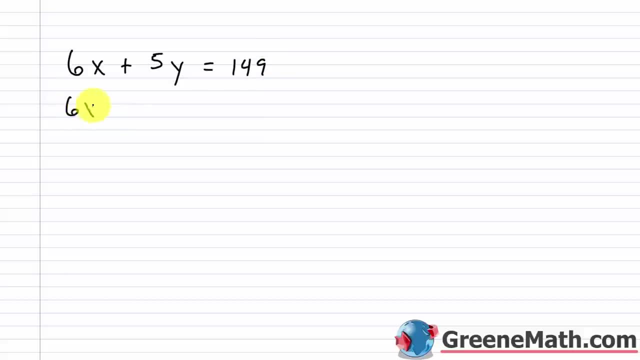 And then I also have six X plus two Y equals 92. Now, it'll probably be easiest to use elimination here. Now, none of my variables would drop out if I just went through and started adding. What I need to do is make a slight modification. You can see that the coefficient of X is six here and six here. So if I multiplied one of these equations, both sides by negative one, one of these would turn into negative six, and one would be positive six. And so when we did our addition, the X variable would drop out. So I'm going to multiply this second equation here by negative one. 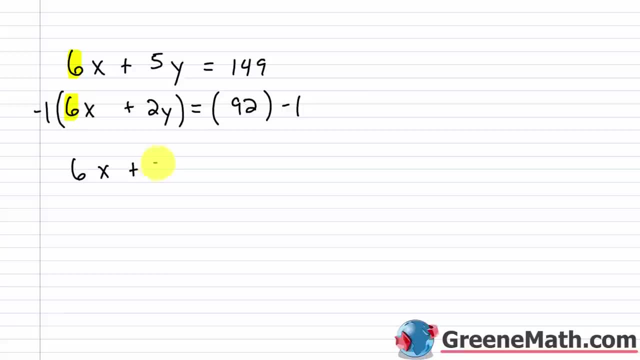 And so I would have six X plus five Y equals 149. Still for my first equation. For my second equation, negative one times six X is negative six X. Then negative one times two Y is minus two Y. 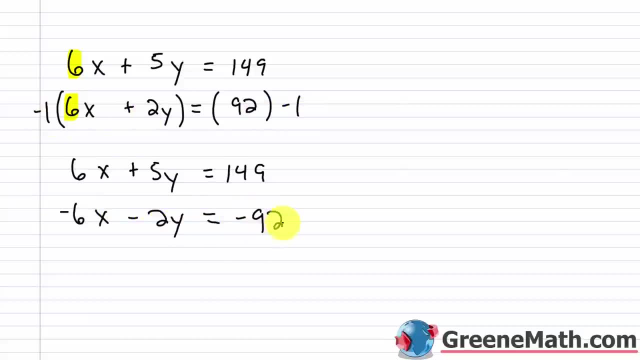 And this equals negative one times 92. That's negative 92. All right, so let's add the two left sides together. 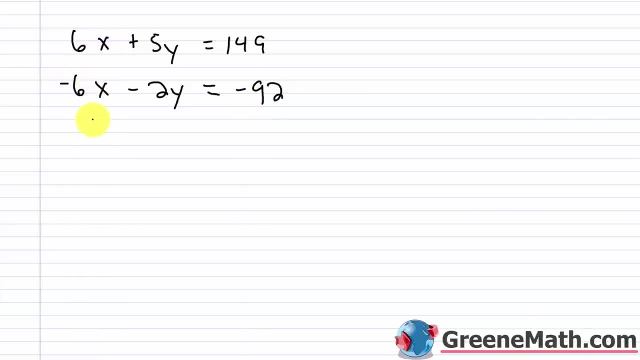 So I'm going to do this vertically. So six X plus negative six X is zero. So that's been eliminated. 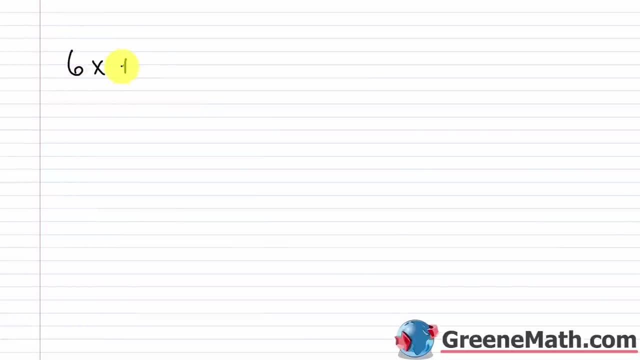 down here. so i have 6x plus 5y- equals 149, and then i also have 6x plus 2y- equals 92. now it'll probably be easiest to use elimination here. now. none of my variables would drop out if i just went through and started adding. what i need to do is make a slight 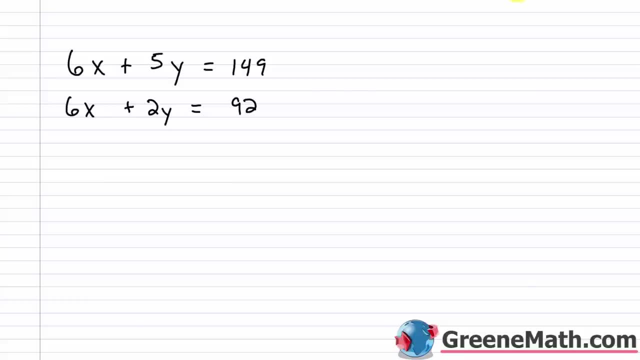 modification, you can see that the coefficient of x is six here and six here. so if i multiplied one of these equations, both sides, by negative one, one of these would turn into negative six and one would be positive six, and so when we did our addition, we would get a negative six. 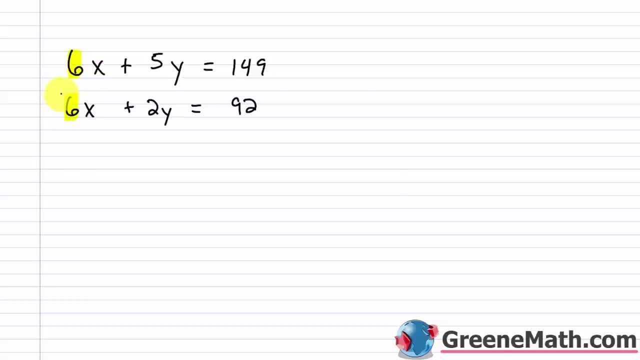 in addition, the x variable would drop out. so i'm going to multiply this second equation here by negative one, and so i would have 6x plus 5y equals 149. still for my first equation. for my second equation: negative one times 6x is negative 6x, then negative one times 2y is minus 2y, and this: 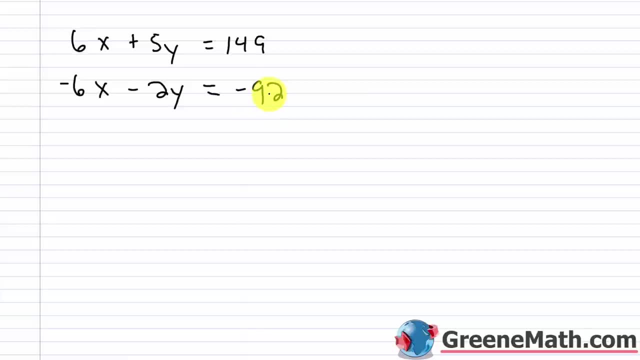 equals negative one times 92. that's negative 92. all right, so let's add the two left sides together. so i'm going to do this vertically. so 6x plus negative 6x is zero, so that's been eliminated. 5y minus 2y is 3y, and this equals- now we're going to sum the right sides- 149 plus negative 92. 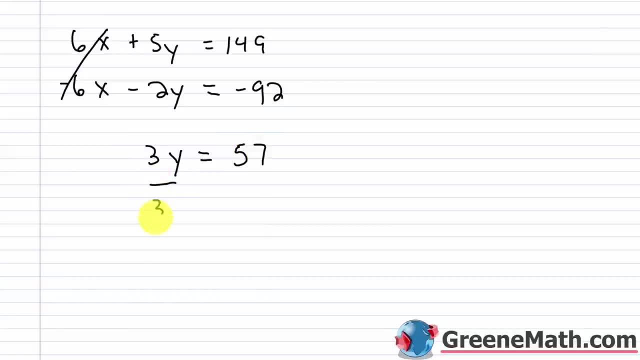 is 57.. so the final step: we divide both sides of the equation by three and we get that y is equal to 19.. so once you have this, you're not done, you need to figure out a value for x, and we look at our two original equations again: y is equal to 19. 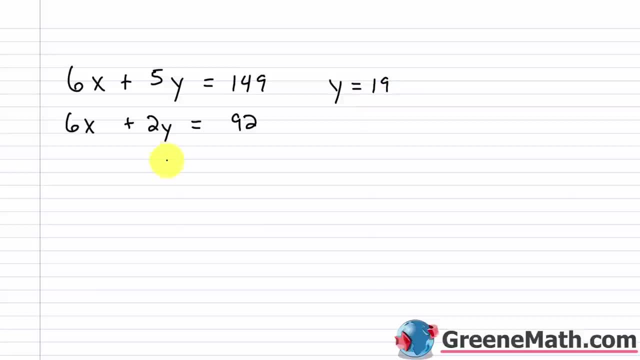 i can plug a 19 in for y in either equation. looks like it'll be a little bit easier here. so i'd have: 6x plus 2 times 19 is equal to 92.. so then this is: 6x plus 2 times 19 is 38, so 38. 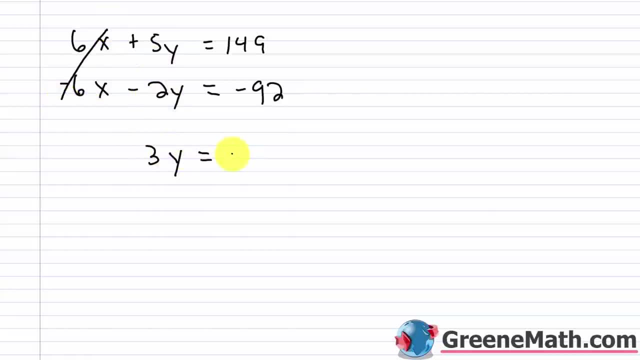 Five Y minus two Y is three Y. And this equals, now we're going to sum the right sides. 149 plus 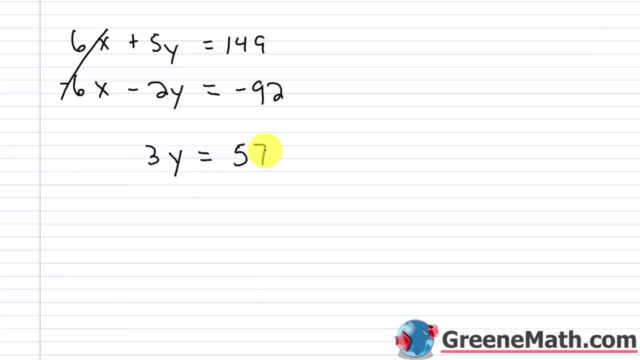 negative 92 is 57. So the final step, we divide both sides of the equation by three, and we get 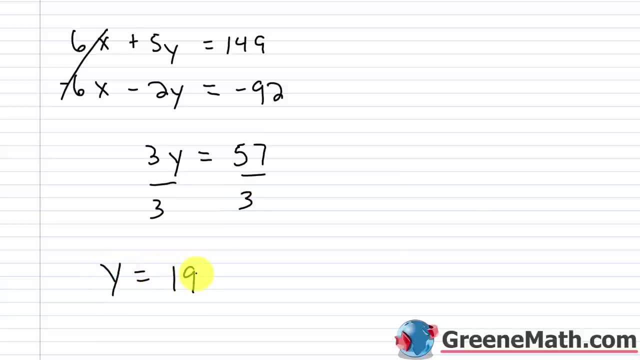 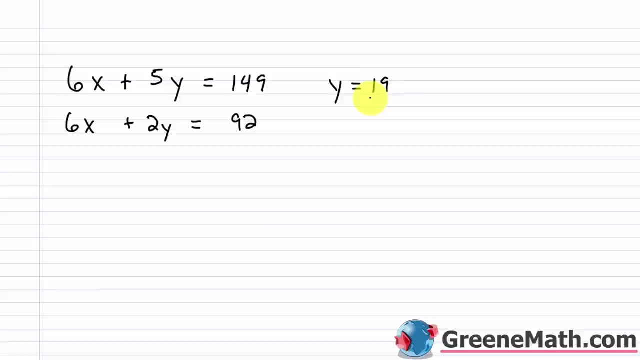 that Y is equal to 19. So once you have this, you're not done. You need to figure out a value for X. And we look at our two original equations. Again, Y is equal to 19. So we plug a 19 in for Y in either equation. Looks like it'll be a little bit easier here. So I'd have six X plus two times 19 is equal to 92. So then this is six X plus two times 19 is 38. 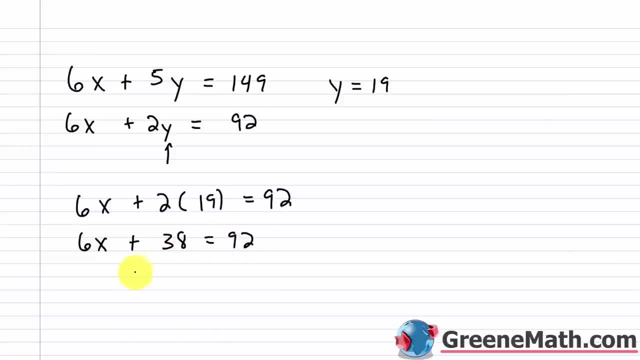 So 38 equals 92. Subtract 38 away from each side of the equation. That's going to cancel. I'll have six X is equal to 92 minus 38 is 54. And then we divide both sides of the equation by six. 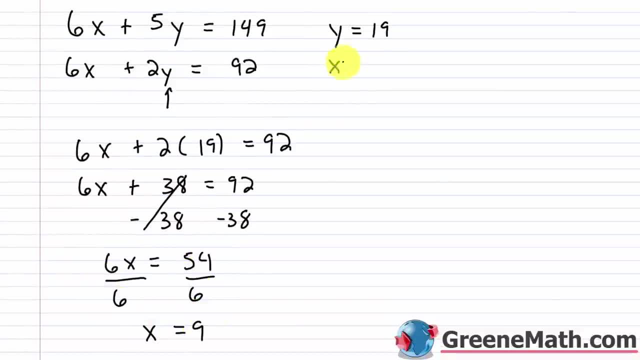 We get that X is equal to nine. So this is the ordered pair, nine comma 19. And just for the sake of completeness, I like to go through and check, make sure that that ordered pair works as a solution to both equations. And then we go back up and then we state our answer. So nine is X. So six times nine plus five times 19 is my value for Y. And this should equal 149. Six times 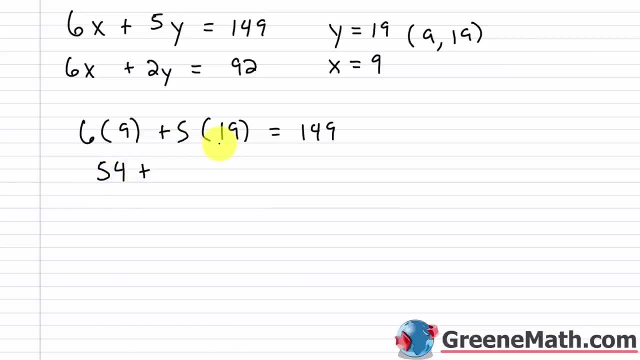 nine is 54 plus five times 19 is 95. So this should equal 149. And it does. You get 149 equals 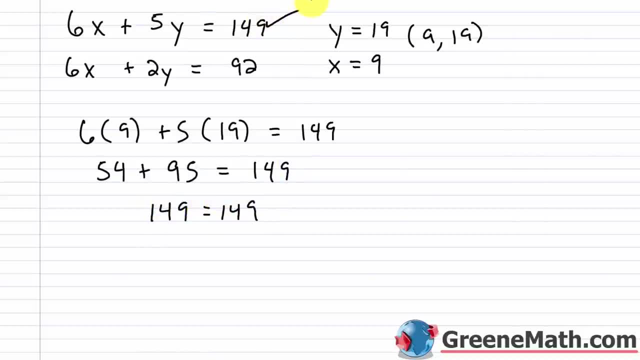 149. So we're good to go here. Let's look at the second equation. All right, for the second one, we're going to, again, plug in a nine for X. So we'd have six times nine. 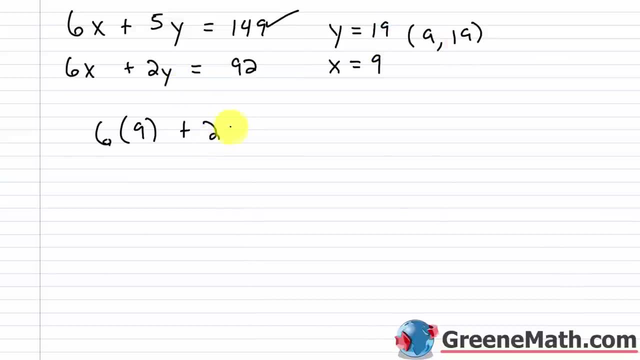 Plus two times for Y we're plugging in a 19. And this should equal 92. Six times nine again is 54 plus two times 19. That's 38. This should equal 92. And 54 plus 38 is 92. So you get 92 equals 92. 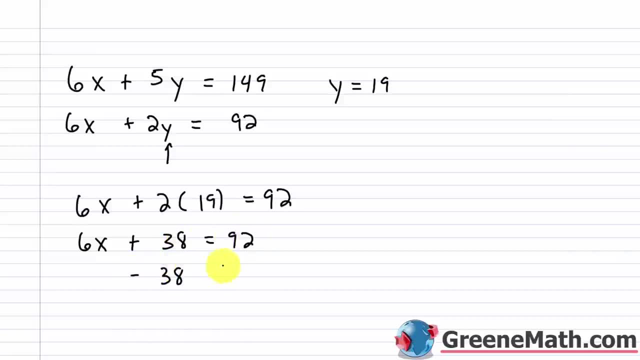 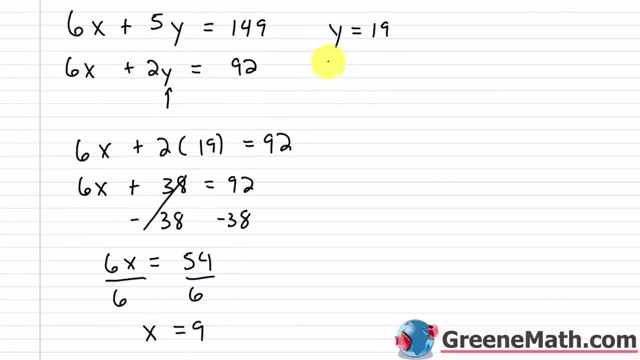 equals 92.. subtract 38 away from each side of the equation. that's going to cancel, i'll have 6x is equal to 92, minus 38 is 54. and then we divide both sides of the equation by 6 and we get that x is equal to 9.. so this is the ordered pair 9, comma 19.. and just for the: 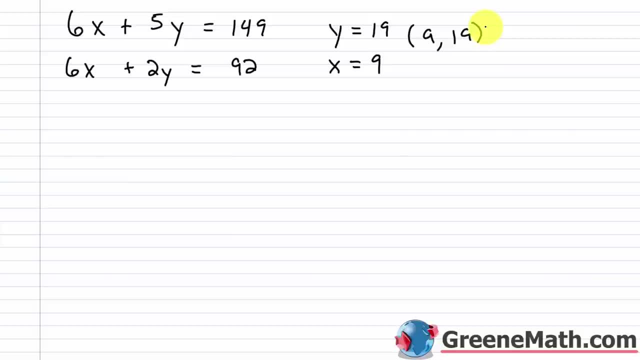 sake of completeness, i like to go through and check, make sure that that ordered pair works as a solution to both equations and then we go back up and then we state our answer. so 9 is my value for x. so 6 times 9 plus 5 times 19 is my value for y, and this should equal 140. 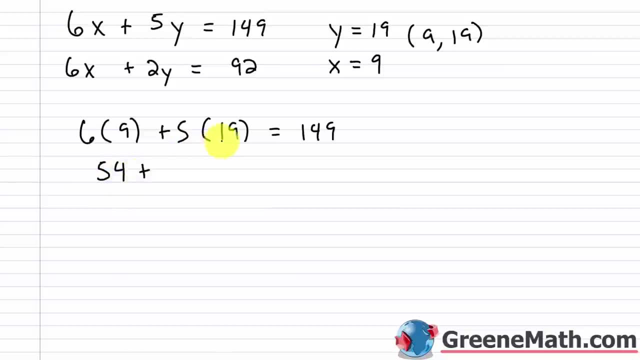 6 times 9 is 54, plus 5 times 19 is 95. so this should equal 149, and it does you get. 149 equals 149, so we're good to go here. let's look at the second equation. all right for the second one. 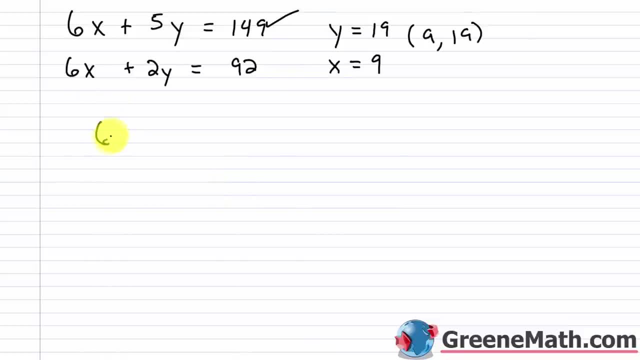 we're going to again plug in a 9 for x, so we'd have 6 times 9 plus 2 times for y, we're plugging in a 19, and this should equal 92.. so we're going to plug in a 9 for x, so we'd have 6 times 9 plus 2 times for y, we're plugging in a 19, and this should equal 92.. 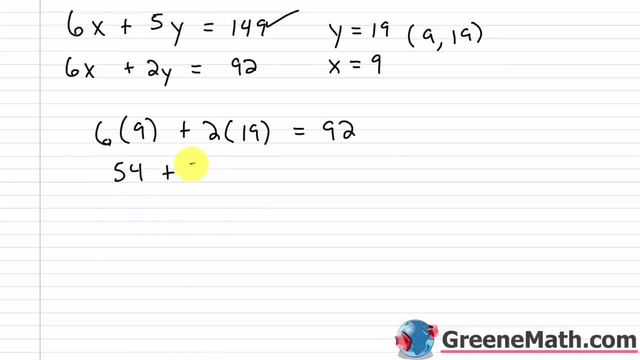 6 times 9 again is 54, plus 2 times 19, that's 38. this should equal 92, and 54 plus 38 is 92. so you get 92 equals 92. so yeah, checks out here as well. now remember, with a word problem you've got to make. 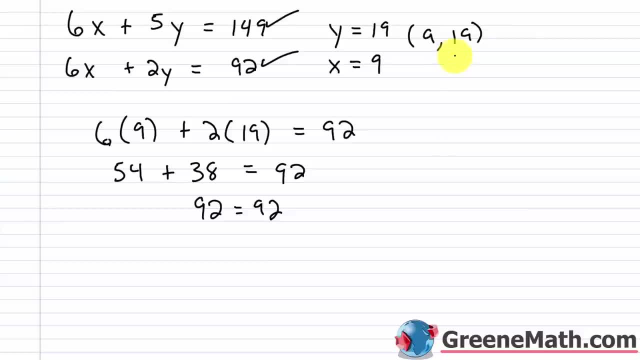 sense of everything. you can't just stop and say: my answer is the ordered pair 9, comma 19.. that doesn't relate to what you got. your teacher would only probably give you partial credit for that. so let's go back up to where we wrote what the variables were representing. 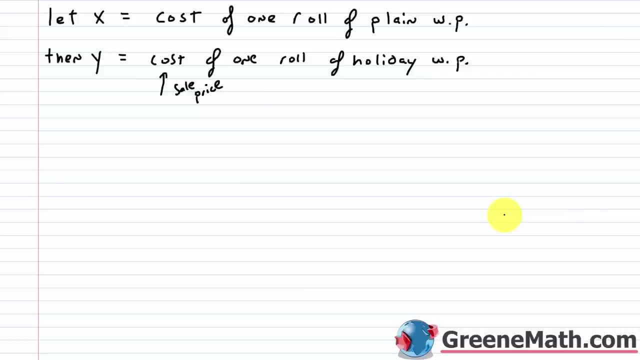 so remember, x was the cost, or again the sale price, of one roll of plain wrapping paper, and we found that x was equal to nine. so x was equal to nine. so then one roll of plain wrapping paper is nine dollars. then y is the cost of one roll of holiday wrapping paper. we found that y was 19. 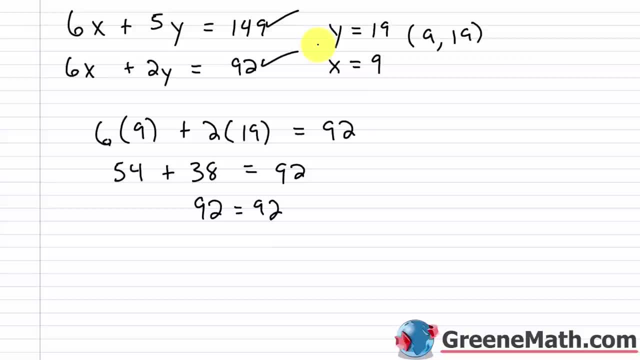 So yeah, checks out here as well. Now remember with a word problem, you've got to make sense of everything. You can't just stop and say, my answer is the ordered pair, nine comma 19. That doesn't relate to what you got. Your teacher, would only probably give you partial credit for that. So let's go back up to where we wrote what 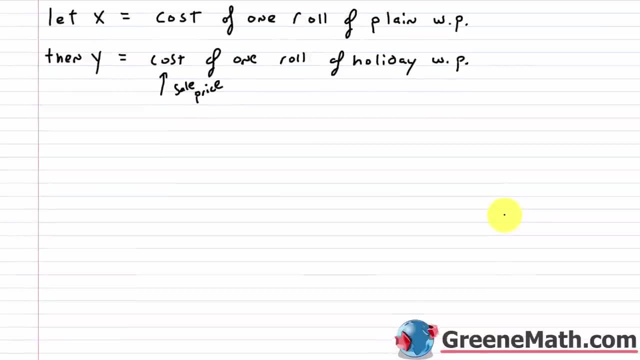 the variables were representing. So remember X was the cost or again, the sale price of one roll of plain wrapping paper. And we found that X was equal to nine. So X was equal to nine. So then one roll of plain wrapping paper is $9. Then Y is the cost of one roll of holiday wrapping paper. We found that Y was $19. 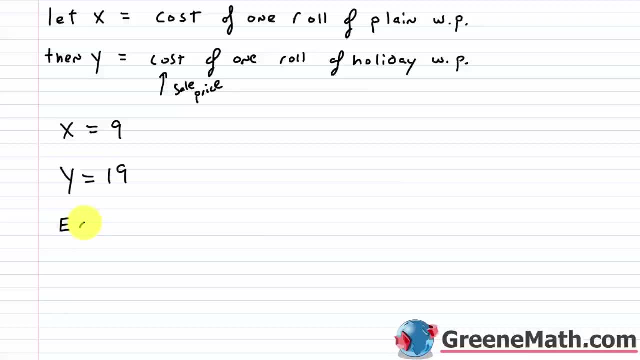 So to answer this, we can say that each roll of plain wrapping paper, which again, I'll abbreviate, sells for $9 while each roll of holiday wrapping paper sells 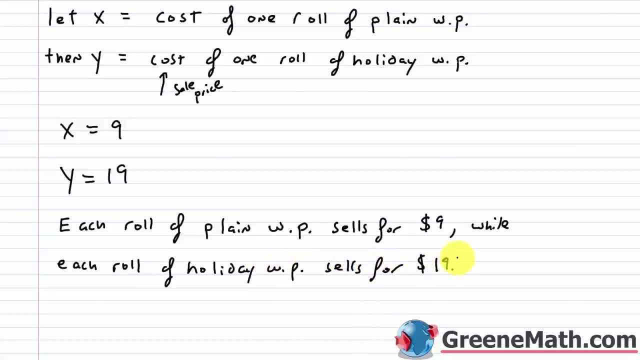 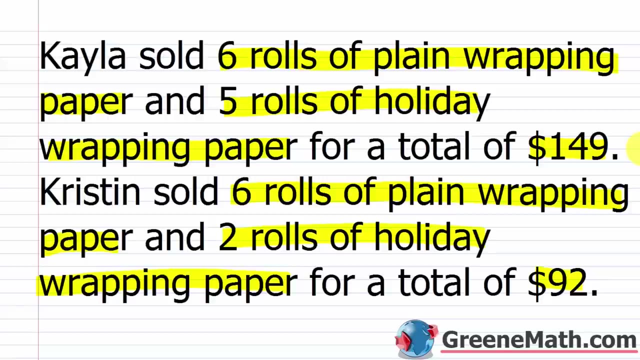 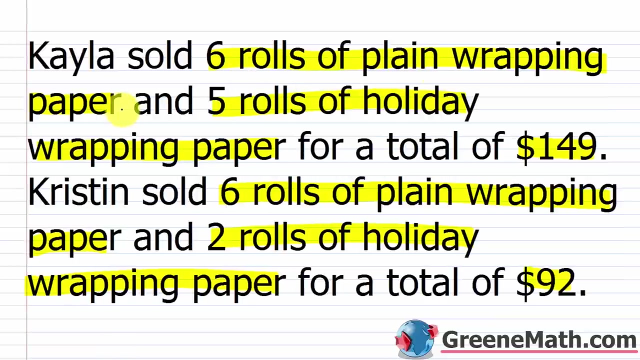 for $19. And although we've checked the equations, go back into your actual problem and make sure that that makes sense. So again, Kayla sold six rolls of plain wrapping paper and five rolls of holiday wrapping paper for a total of $149. So you're checking this just like you checked your equation. It's basically the same thing. So six rolls of plain wrapping paper. Again, each roll is $9. So that would be $54. And five rolls of holiday wrapping paper. Again, each roll is $19. Five times 19 is 95. So you sum these two amounts together, you would get a total of $149. 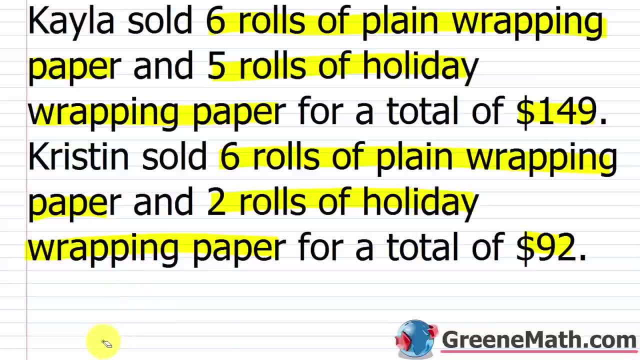 So that part's good to go. Then again, the second part, Kristen sold six rolls of plain wrapping paper. Six times, again, nine is 54. So that's $54. Two rolls of holiday wrapping paper, $229. And again, the second part, Kristen sold six rolls of plain wrapping paper. So that's $54. So that's $54. Two rolls of holiday wrapping paper, $229. And again, the second part, Kristen sold six rolls of plain wrapping paper, $229. And again, the second part, Kristen sold six rolls of holiday wrapping paper, $229. And again, the second part, Kristen sold six rolls of 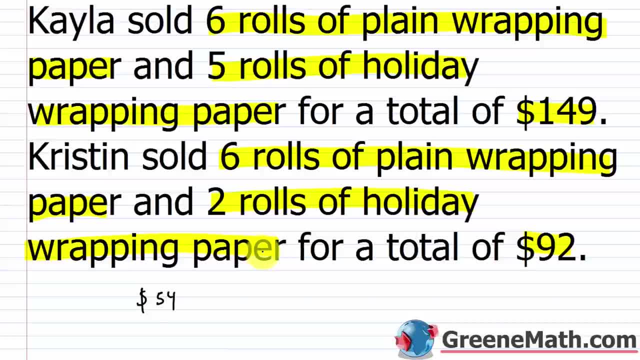 $19. Right, $19 a piece for the holiday wrapping paper, that's $38. Sum these two amounts together and you would in fact get $92. So our answer here is correct. Each roll of plain wrapping paper sells for $9. And each roll of holiday wrapping paper is going to sell for $19. 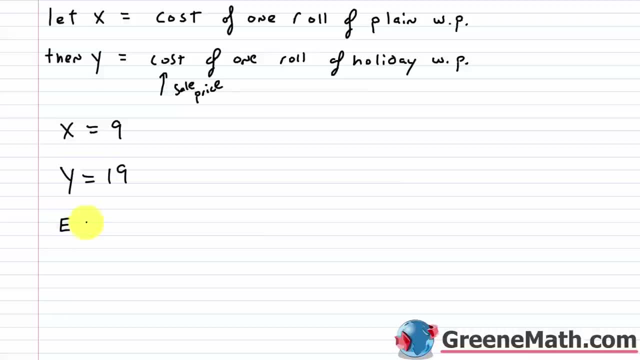 so to answer this, we can say that each roll of plain wrapping paper- which again i'll abbreviate- sells for nine dollars, while each roll of holiday wrapping paper sells for nineteen dollars. and although we've checked the equations, go back into your actual problem and make sure that that makes sense. so again, kayla sold six rolls of plain. 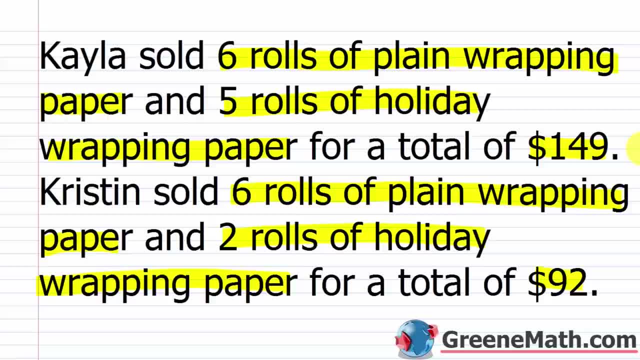 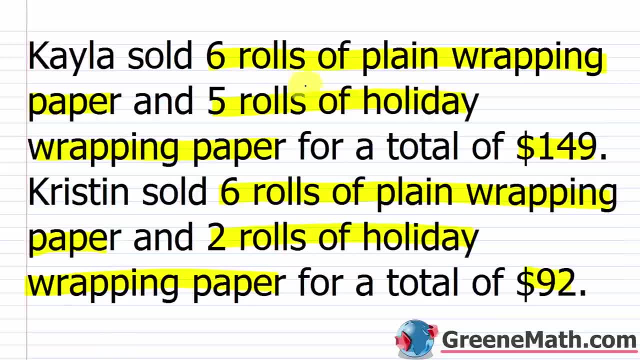 wrapping paper and five rolls of holiday wrapping paper for a total of 149 dollars. so you're checking this just like you checked your equation. it's basically the same thing. so six rolls of plain wrapping paper- again, each roll is nine dollars. so that would be fifty four dollars. 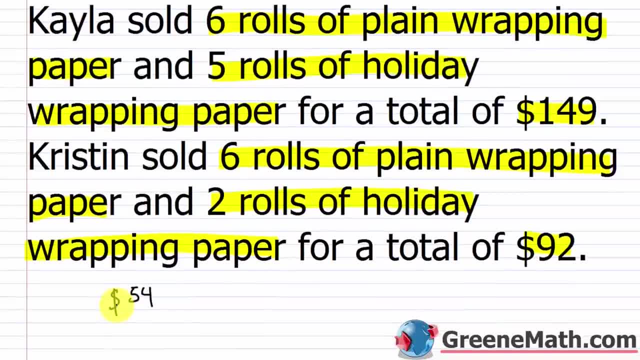 and five rolls of holiday wrapping paper. again, each roll is nineteen dollars. five times 19 is 95. so you sum these two amounts together you would get a total of 149 dollars. so that part's good to go. then again the second part. kristen sold six rolls of plain wrapping paper. 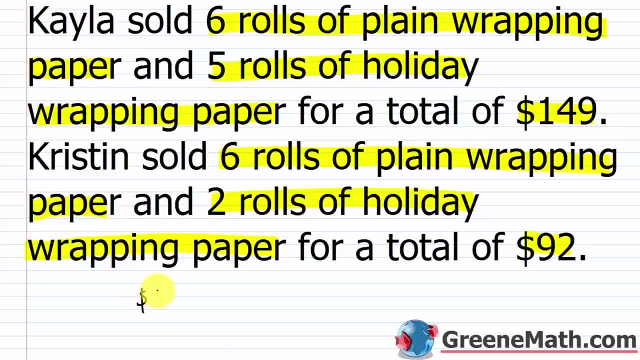 six times again nine is 54, so that's 54 dollars. two rolls of holiday wrapping paper two times 19 right 19 a piece for the holiday wrapping paper. that's 38 dollars. sum these two amounts together and you would in fact get 92 dollars. so our answer here is correct. 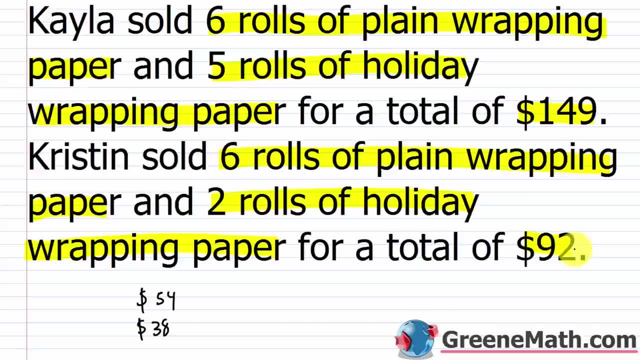 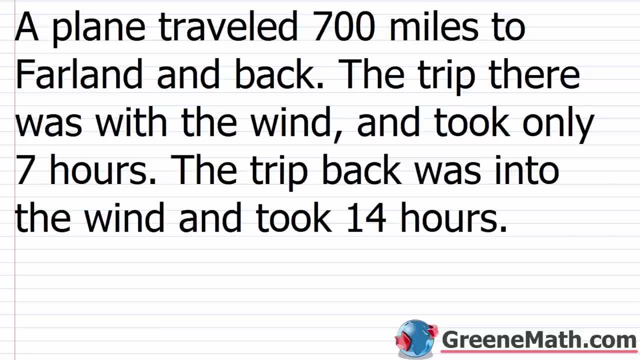 each roll of plain wrapping paper sells for nine dollars, and each roll of holiday wrapping paper is going to sell for 19 dollars. all right, let's take a look at another one. so a plane traveled 700 miles to far land and back. the trip there was with the wind and took only seven hours. 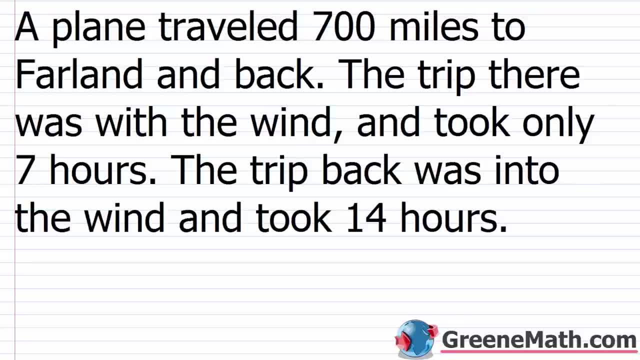 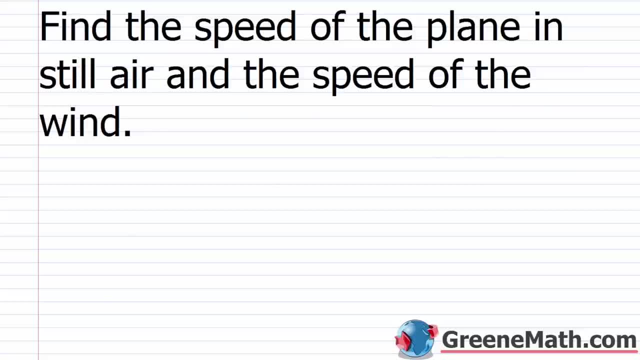 the trip back was into the wind and took 14 hours. find the speed of the plane in still air and the speed of the wind. so when you get these type of problems, you're always thinking about okay, although it might not be a hundred percent accurate in real life. 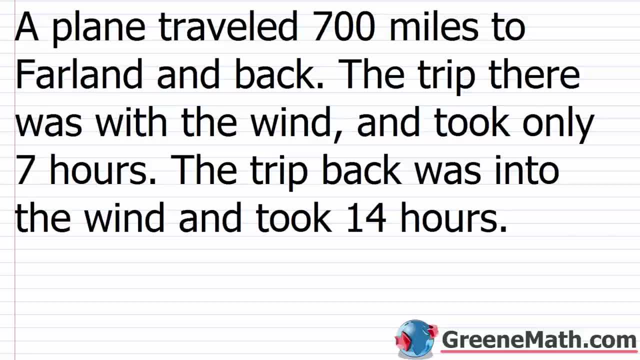 All right, let's take a look at another one. So a plane traveled 700 miles to far land and back. The trip there was with the wind and took only seven hours. The trip back was into the wind and took 14 hours. Find the speed of the plane in still air 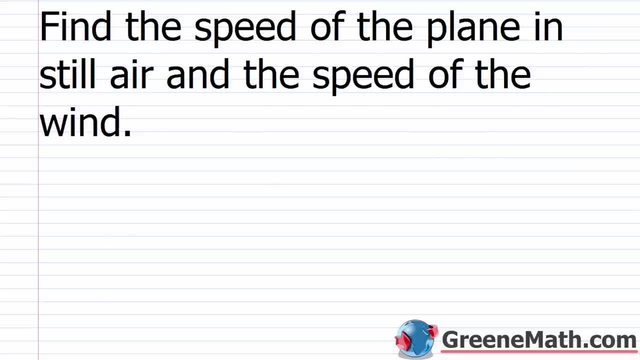 and the speed of the wind. So when you get these type of problems, you're always thinking about, okay, although it might not be 100% accurate in real life, if you're going with the wind, the wind is pushing on the back of the plane. Or a lot of times you'll see these with a kind of a current problem where the current is pushing the boat. So you have a current or you have a wind that's pushing at your back. So you have a current or you have a wind that's pushing at your back. That's making you go faster. When you fly into the wind or when you are in a boat and you go against the current, you're fighting it. So you're going slower. So the main thing you're trying to figure out here, your main objective is to find the speed of the plane in still air. So meaning the air is not moving at all and the speed of the wind. So the speed of the wind. 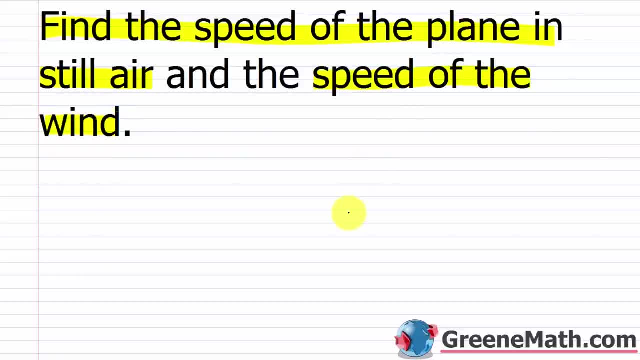 So we're going to use two variables to represent each, right? Those are our two unknowns. So let X equal the speed of the plane in still air. And then Y can be the speed of the wind. 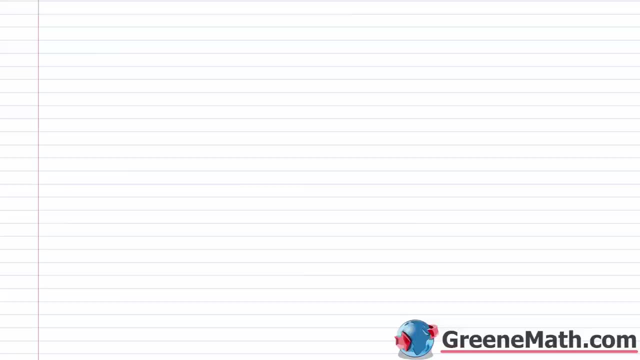 Now, again, for this type of problem, because it involves motion, we're going to be using our distance formula. So you should remember this from when we were doing the first example. So 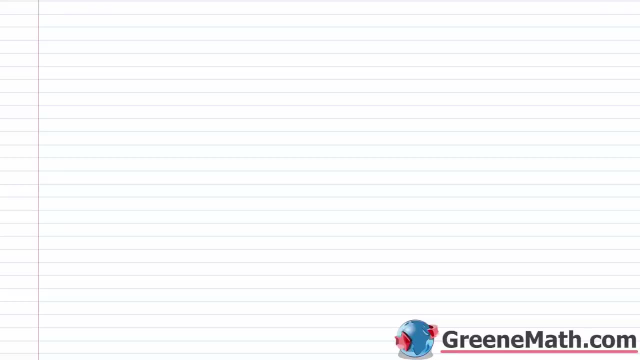 we're solving word problems with linear equations of one variable. The distance formula looks like this. You have your distance is equal to the rate of speed multiplied by the amount of time traveled. 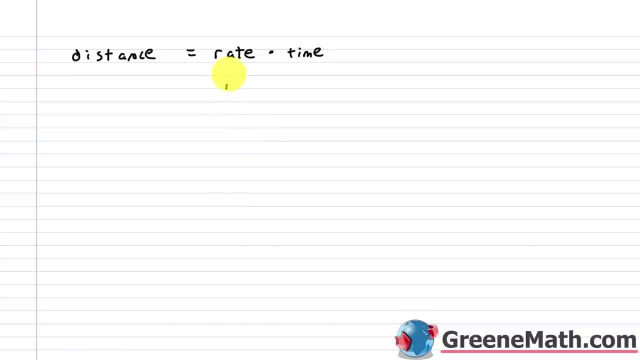 And again, this is very, very intuitive. You jump in a car, you go 70 miles per hour for four hours. Forget about the units, just multiply the numbers together. 70 times the times four is 280. So that would be 280. If you think about the units, it would be 280 miles. 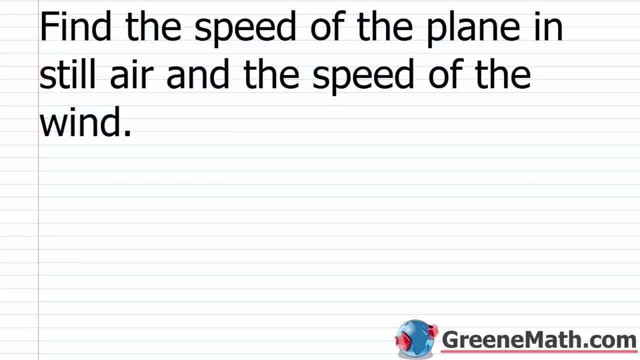 if you're going with the wind, the wind is pushing on the back of the plane, or a lot of times you'll see these with a kind of a current problem, where the current is pushing the boat. so you have a current or you have a wind that's pushing at your back. that's making 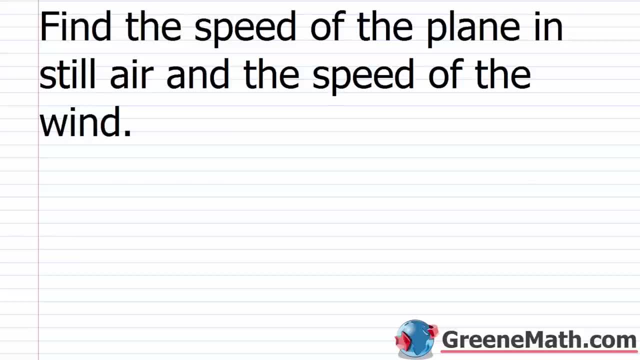 you go faster when you fly into the wind or when you are in a boat and you go against the current. you're fighting it, so you're going slower. So the main thing you're trying to figure out here, your main objective, is to find the speed of the plane in still air. 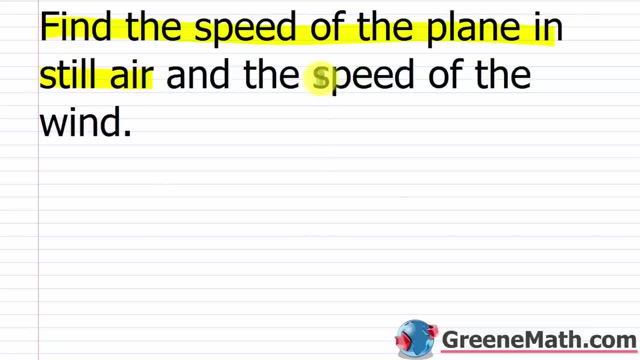 So meaning the air is not moving at all, And the speed of the wind, So the speed of the wind. So we're going to use two variables to represent each right. Those are our two unknowns. So let's let x equal the speed of the plane. 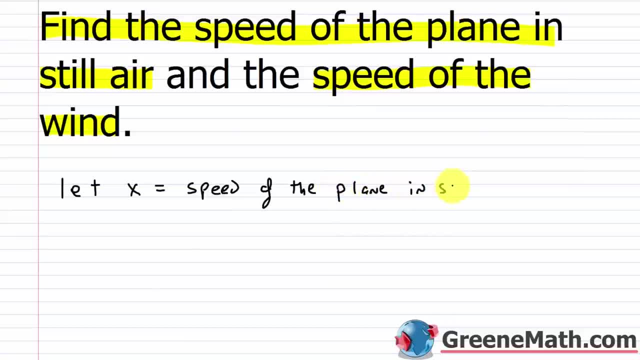 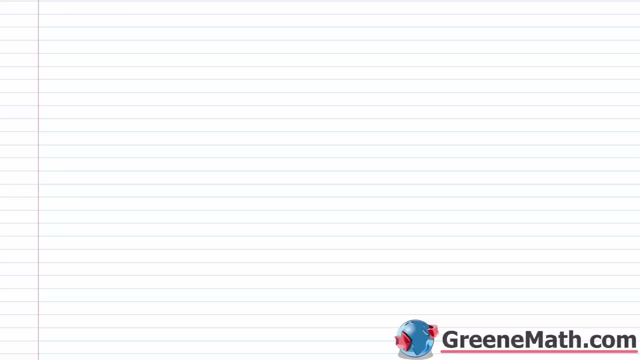 in still air, And then y can be the speed of the wind. Now again, for this type of problem, because it involves motion, we're going to be using our distance formula, So you should remember this from when we were solving word problems. 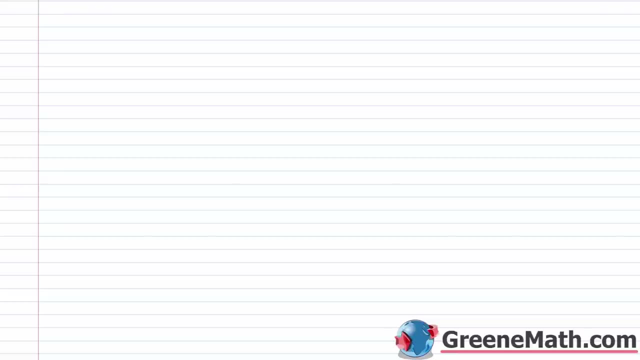 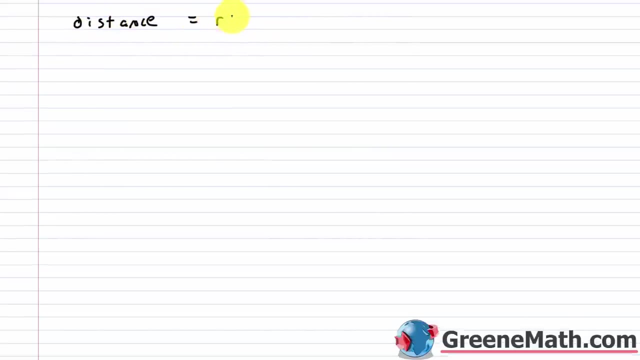 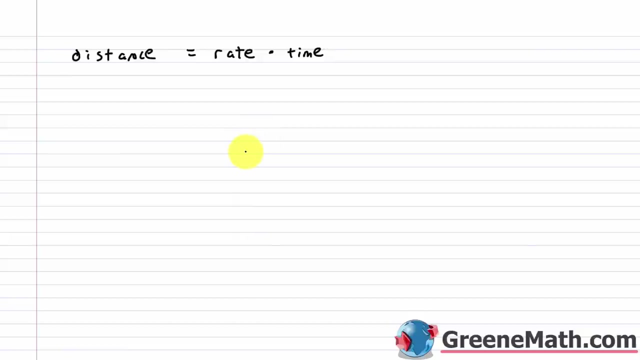 with linear equations of one variable. The distance formula looks like this, You have: your distance is equal to the rate of speed multiplied by the amount of time traveled. And again, this is very, very intuitive. You jump in a car, You go 70 miles per hour. 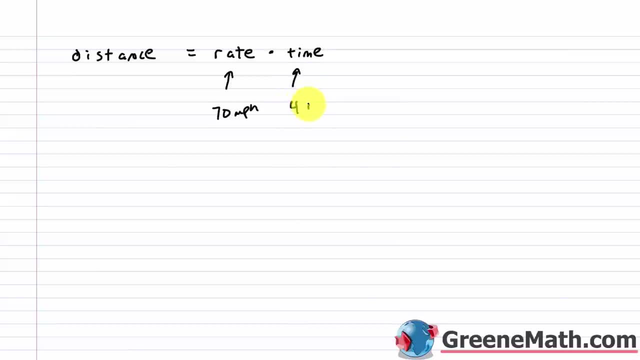 for four hours. Forget about the units. Just multiply the numbers together. 70 times 4 is 280.. So that would be 280.. If you think about the units, it would be 280 miles. Very, very easy to calculate your distance. 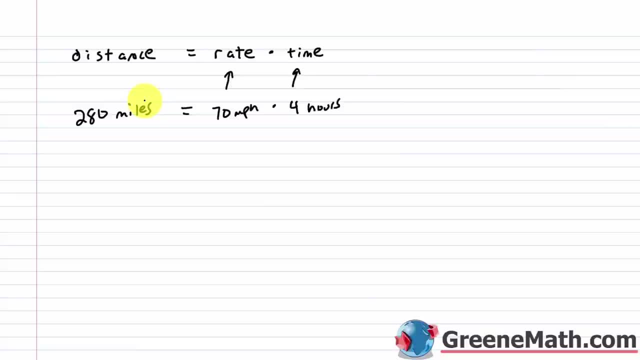 if you know a rate and a time, Just multiply the two together. You could manipulate this in many ways. You could solve for rate and figure that out if you had the time and the distance. Or you could solve for time and figure that out. 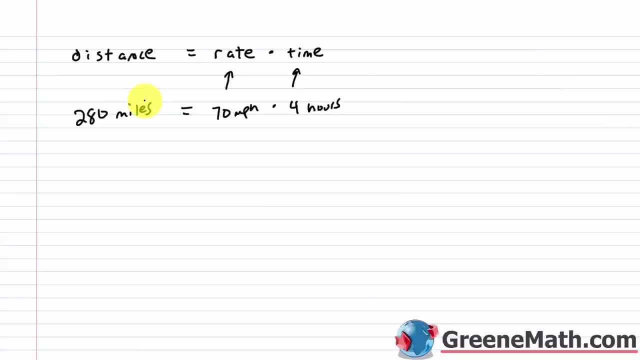 Very, very easy to calculate your distance. If you know a rate and a time, just multiply the two together. You could manipulate this in many ways. You could solve for rate and figure that out. If you had the time and the distance where you could solve for time and figure that out, if you had the rate and the distance, right? So on and so forth. But what we're going to do in this particular 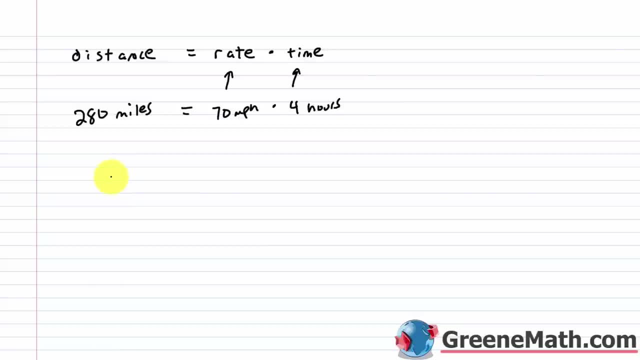 problem is set up a nice little table. So I have that distance is equal to rate times time. So I'm going to put this up top, draw a little line down here. All right. So we have two scenarios. We have the trip there. 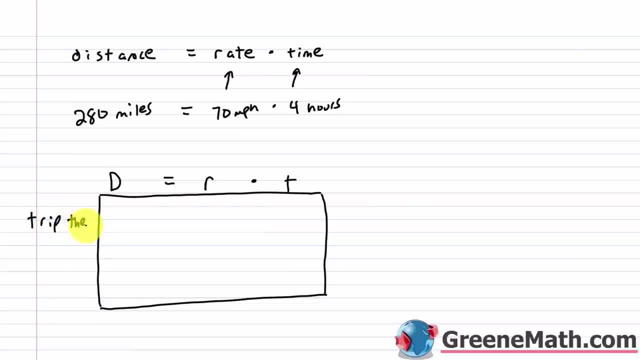 We have the trip there. And we have the trip back. Let me get a little bit more room. Let me kind of scoot this over. 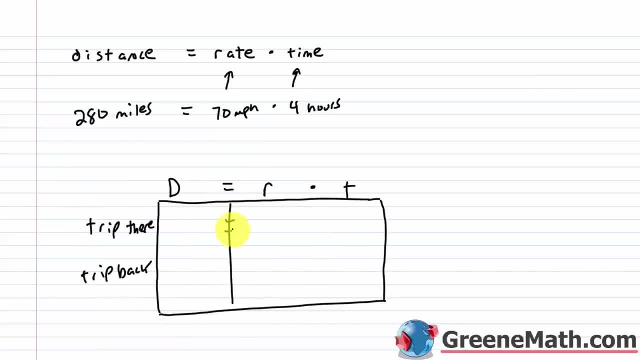 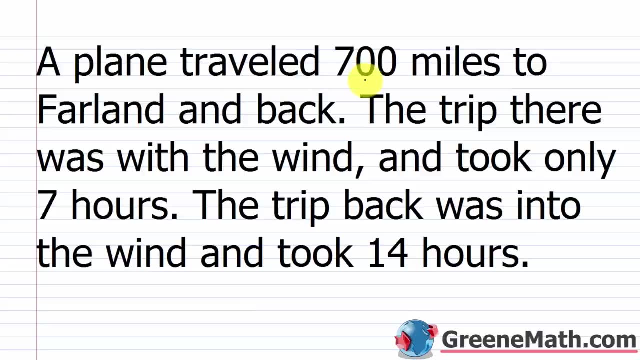 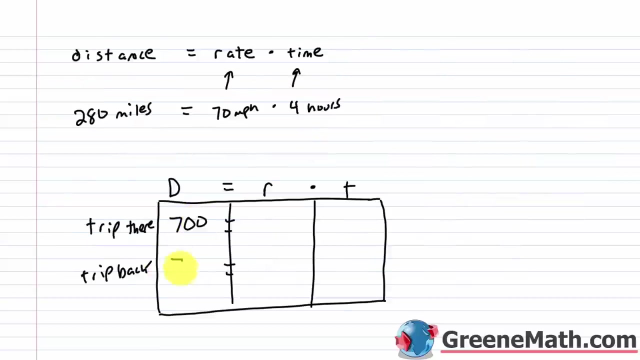 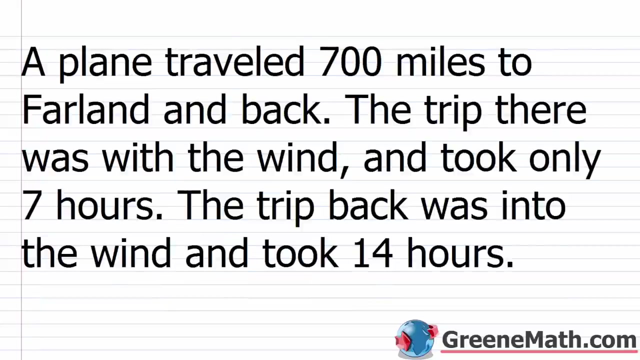 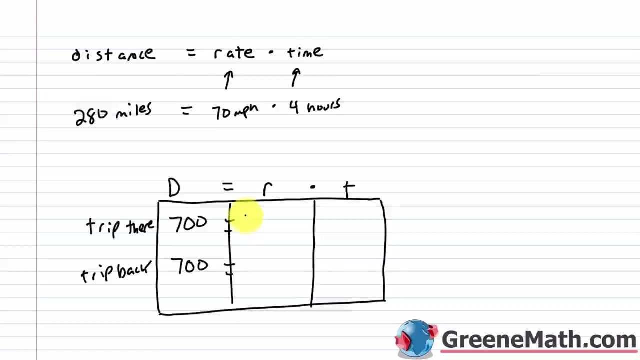 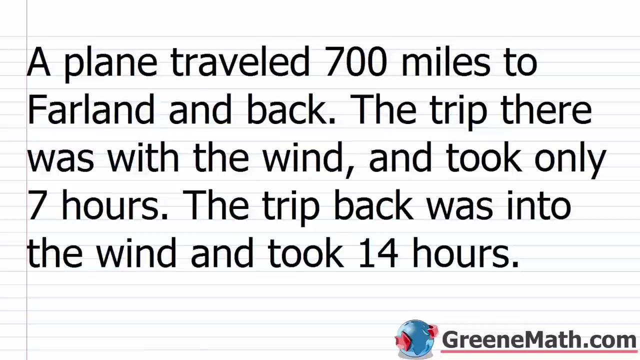 All right. So let me put this down here. Equals, equals. So let's go on and get some information. So for the trip there, we know the distance is 700 miles in each case. So the trip there and the trip back, the plane traveled 700 miles to Farland and back. So the distances will be the same. So let's fill that out. So the trip there, the distance is 700. The trip back, the distance is also 700. Now let's talk about the rate. The trip there was with, the wind. So that means that whatever the plane would do, in terms of its speed, you have to add to that the fact that the wind is pushing at your back. So you take the plane's speed in still air, which we represented with X, and you would add to that the speed of the wind, which we represented with Y. So for your rate for the trip there, it's going to be X plus Y. Now in terms of time, it says, only seven hours. So we have a rate, we have a time, and we have a distance. So the time is seven. 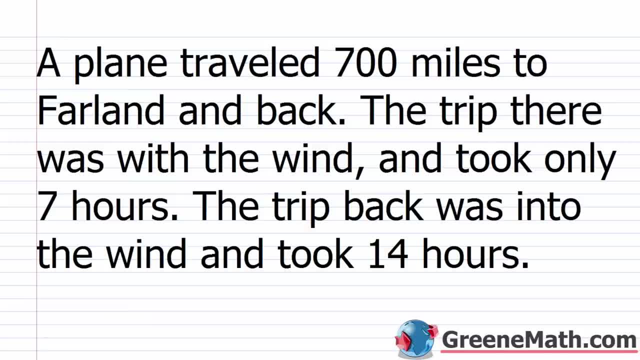 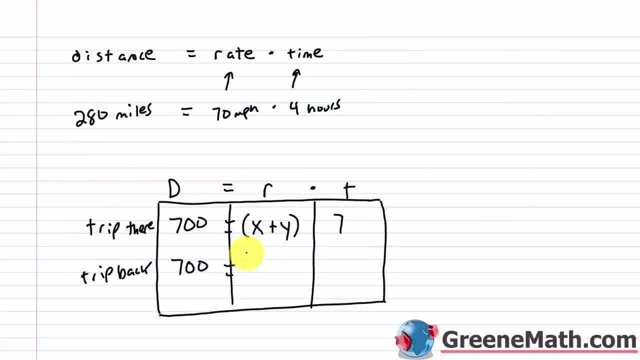 Now for the trip back, it says it was into the wind and it took 14 hours. So into the wind, that means that I'm taking the speed of the plane in still air, which is X, and I'm subtracting away the air speed or the speed of the wind. So that's minus Y. And then the time is 14, right? For 14 hours. So then we'll have our two, 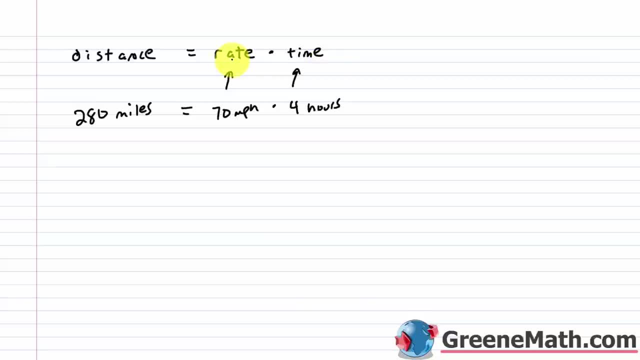 if you had the rate and the distance right, So on and so forth. But what we're going to do in this particular problem is set up a nice little table. So I have that. distance is equal to rate time, times, time. 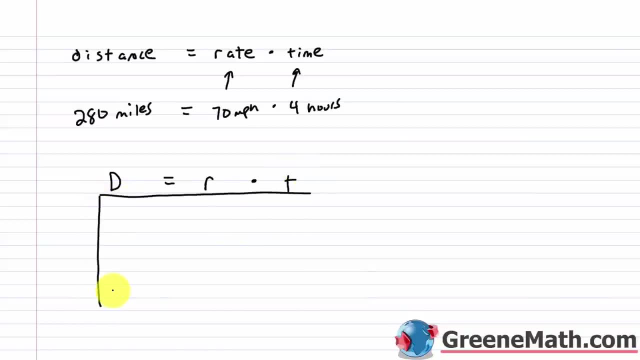 So I'm going to put this up top, Draw a little line down here, All right, so we have two scenarios: We have the trip there, We have the trip there And we have the trip back. Let me get a little bit more room. 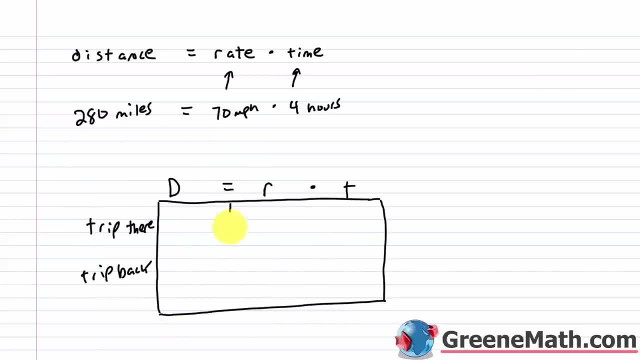 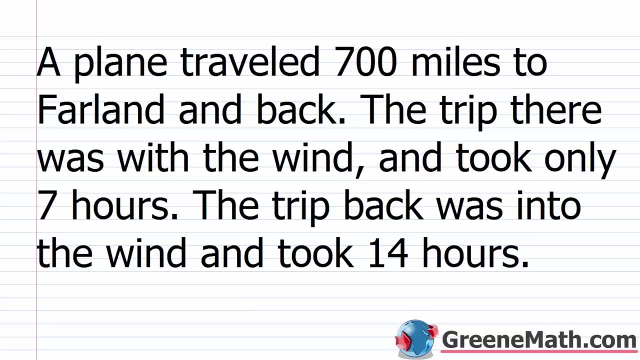 Let me kind of scoot this over, All right. so let me put this down here: Equals equals, So let's go on and get some information. So for the trip there, we know the distance is 700 miles in each case. 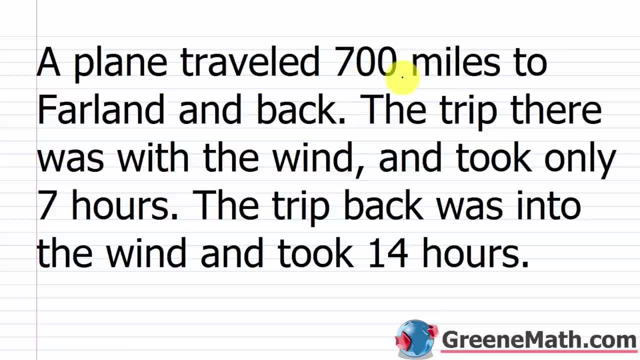 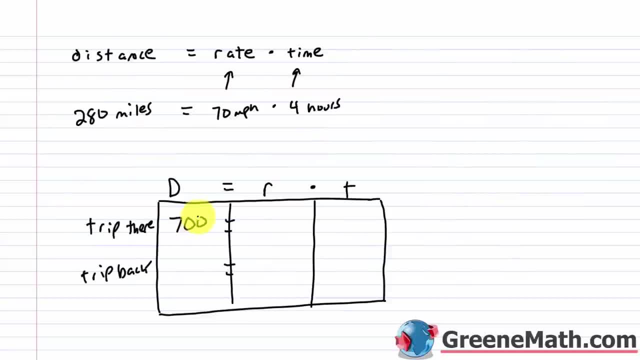 So the trip there and the trip back, the plane traveled 700 miles to Farland and back, So the distances will be the same. So let's fill that out. So the trip there, the distance is 700.. The trip back, the distance is also 700. 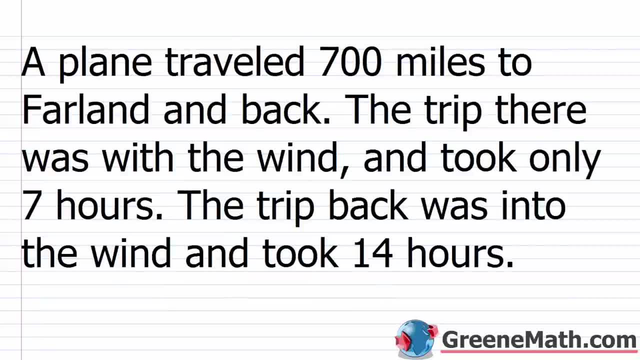 Now let's talk about the rate. The trip there was with the wind. So that means that whatever the plane would do in terms of its speed, you have to add to that the fact that the wind is pushing at your back, So you take the plane's speed in still air. 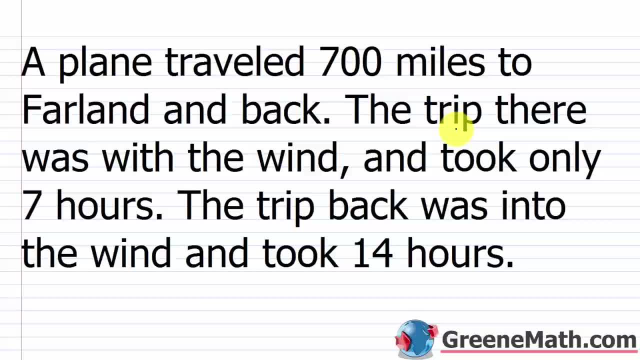 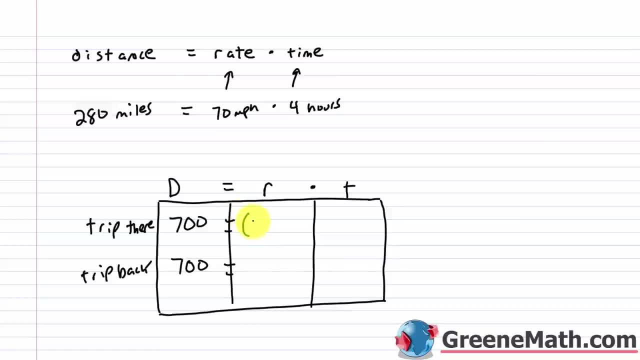 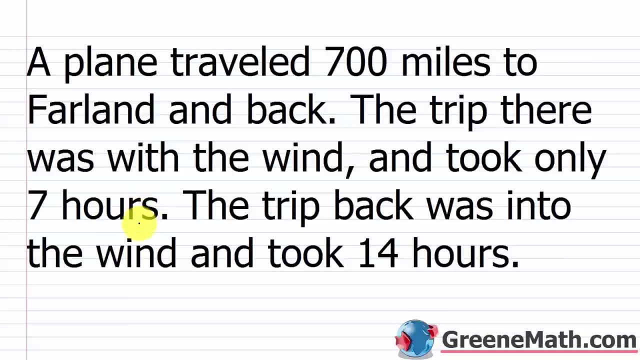 which we represented with X, and you would add to that the speed of the wind, which we represented with Y. So for your rate for the trip there, it's gonna be X plus Y. Now, in terms of time, it says it took only seven hours. 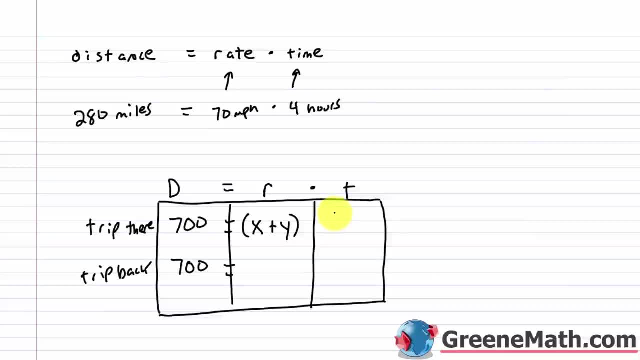 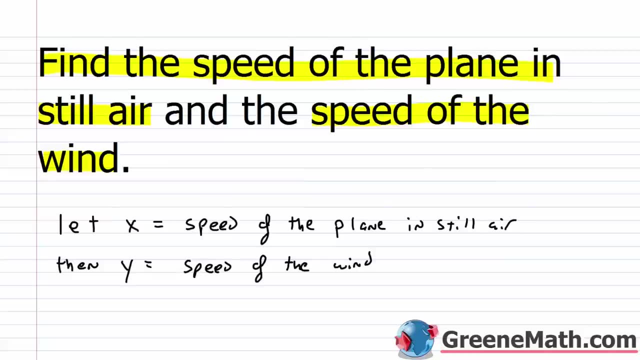 So we have a rate, we have a time and we have a distance. So the time is seven. Now for the trip back. it says it was into the wind and it took 14 hours. So into the wind. that means that I'm taking the speed. 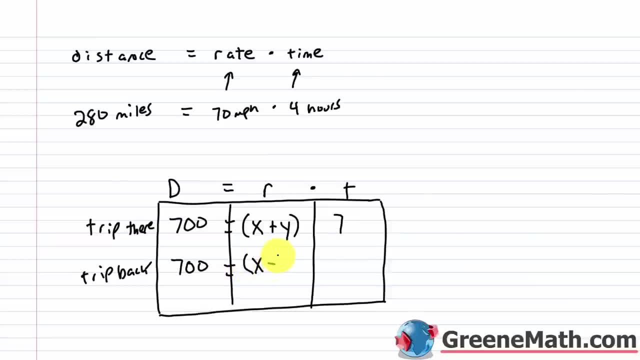 of the plane in still air, which is X, and I'm subtracting away the air speed or the speed of the wind, So that's minus Y, And then the time is 14, right for 14 hours. So then we'll have our two equations. 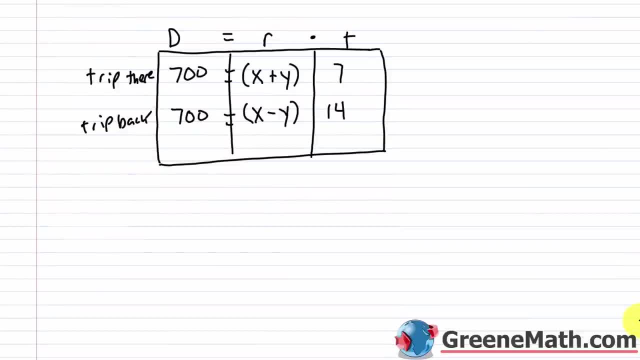 two equations. Essentially, we have an equation for the trip there, which is a rate times a time, we have seven, which is our time, times our rate, which is X. Again, this is the speed of the plane in still air, plus Y, which again is the speed of the wind or the wind speed. And when we multiply these two together, we're going to get the distance, right? This is a time, this is a rate, rate times time gives me a distance. So this should be equal to 700. Then for the trip back, I set up another equation. Again, I have a time that's 14 and this is multiplied by the rate, which is X. Again, the speed of the plane in still air. Now I'm subtracting away the wind speed, because if I'm going against the wind, I'm fighting it. So I got to subtract that away. 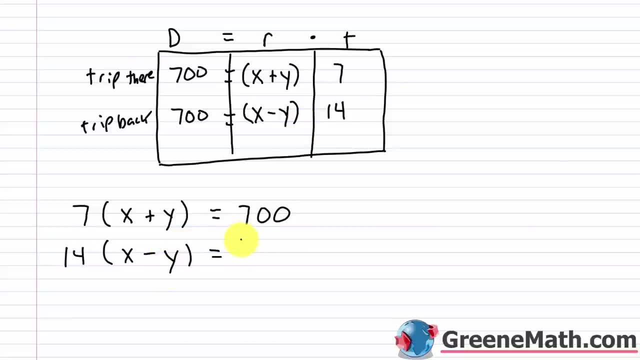 So then minus Y and this equals 700. So I have a time times a rate or a rate times a time gives me a distance. Same thing up here. I have a time times a rate, which is 700. So I have a time times a rate or a rate times a time gives me a distance. Same thing up here. I have a time times a rate, that gives me a distance. So I have two equations and two unknowns. So let's go ahead and just solve 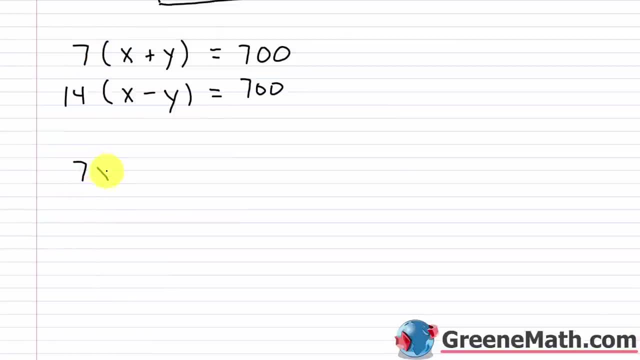 this system. So seven times X is seven X plus seven times Y that's seven Y and this equals 700. And then I have 14 times X that's 14 X and then minus 14 times Y that's 14 Y. And this also equals 700. Now again, it would probably be pretty easy to use the elimination method specifically because I have a negative function and I have a negative function and I have a negative function and I 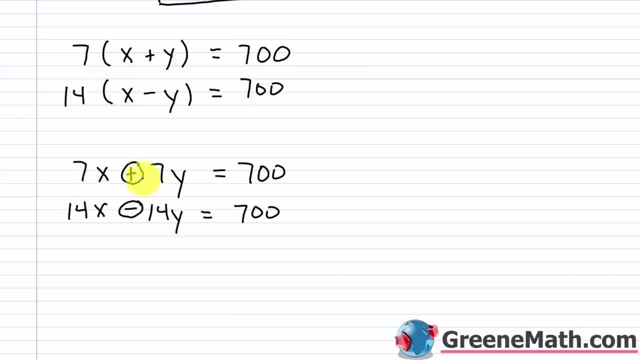 have a positive here and a positive here. And all I need to do is multiply this top equation, both sides by two, and I would have opposite coefficients for my variable Y. So let's go ahead and do that. I multiply this side by two and this side by two. I would have 14 X plus 14 Y is equal to 1400. And I'm going to go ahead and erase this for now. And these are going to be the two equations I work with. So I'm going to use my elimination method. So I'm going to use my elimination method. 14 X plus 14 X is 28 X. When I add here negative 14 Y plus 14 Y, that's going to be eliminated. And then this equals 700 plus 1400, which is 2100 or 2100. So now to get X by itself, 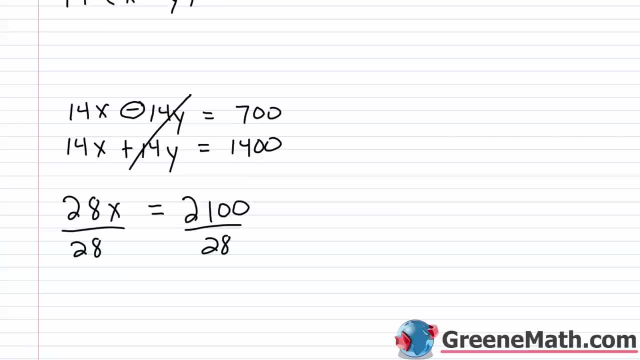 I divide both sides of the equation by 28. And that's going to give me that X is equal to 75. 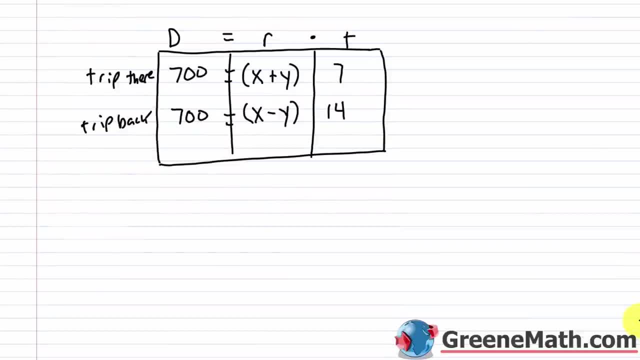 Essentially, we have an equation for the trip there, which is a rate times a time. We have seven, which is our time times our rate, which is X. Again, this is the speed of the plane in still air, plus Y, which again is the speed of the wind. 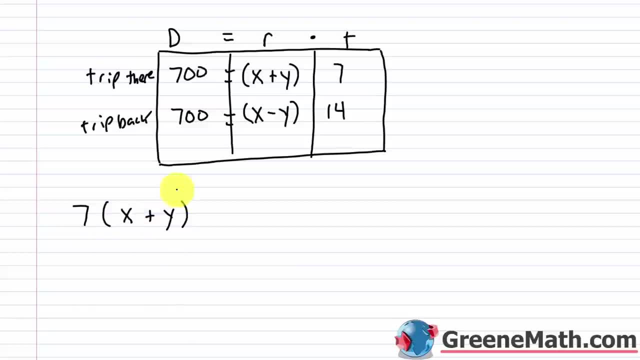 or the wind speed, And when we multiply these two together, we're gonna get the distance right. This is a time. this is a rate Rate times. time gives me a distance, So this should be equal to 700.. Then, for the trip back, I set up another equation. 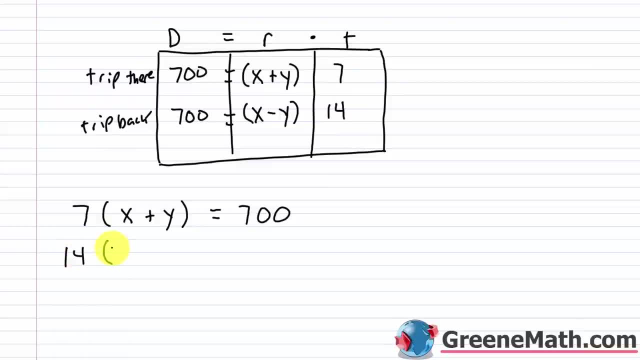 Again, I have a time that's 14.. And this is multiplied by the rate, which is X, Again the speed of the plane in still air. Now I'm subtracting away the wind speed, because if I'm going against the wind, I'm fighting it. 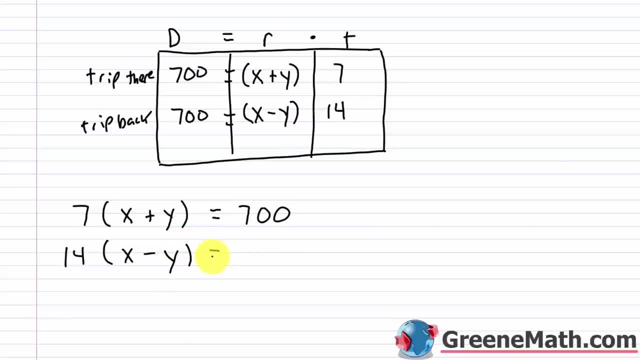 So I gotta subtract that away. So then minus Y and this equals 700.. So I have a time times a rate, or a rate times a time gives me a distance. Same thing up here. I have a time times a rate that gives me a distance. 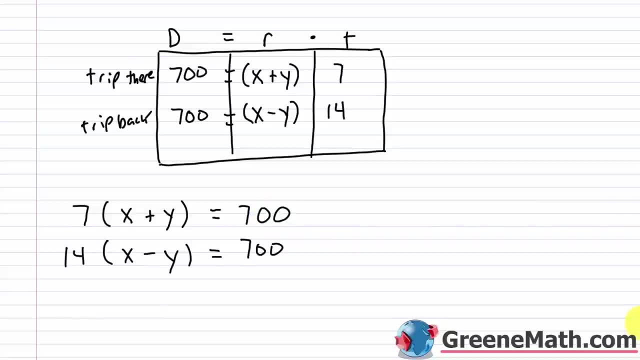 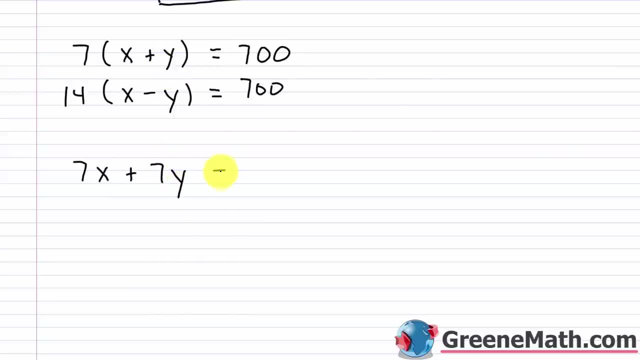 So I have two equations and two unknowns, So let's go ahead and just solve this system. So seven times X is seven X, Plus seven times Y, that's seven Y, And this equals 700.. And then I have 14 times X, that's 14 X. 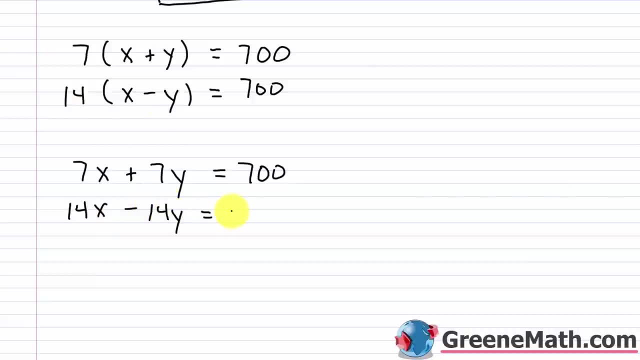 And then minus 14 times Y, that's 14 Y, And this also equals 700.. Now again, it would probably be pretty easy to use the elimination method, specifically because I have a negative here and a positive here And all I need to do is multiply this top equation. 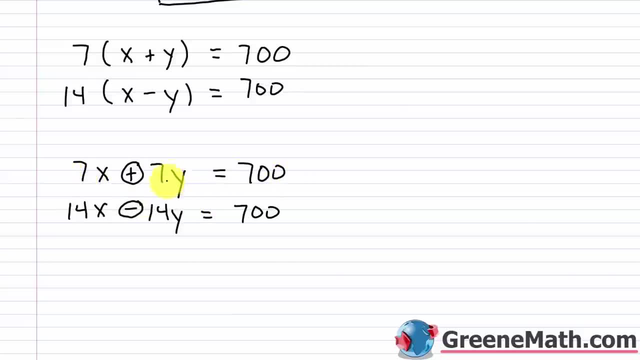 both sides by two and I would have opposite coefficients for my variable Y. So let's go ahead and do that. If I multiply this side by two and this side by two, I would have 14. X plus 14 Y is equal to 1400. 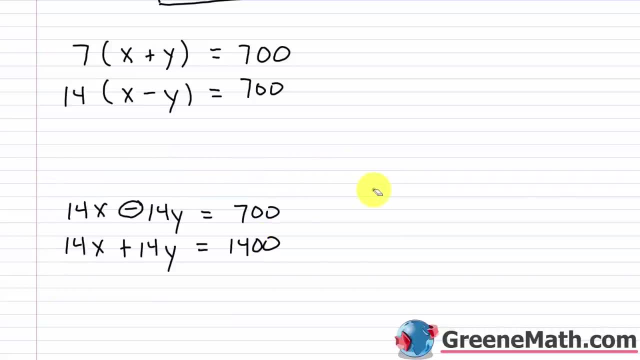 And I'm gonna go ahead and erase this for now, And these are gonna be the two equations I work with, So I'm gonna use my elimination method. 14 X plus 14 X is 28 X When I add here negative 14 Y plus 14 Y. 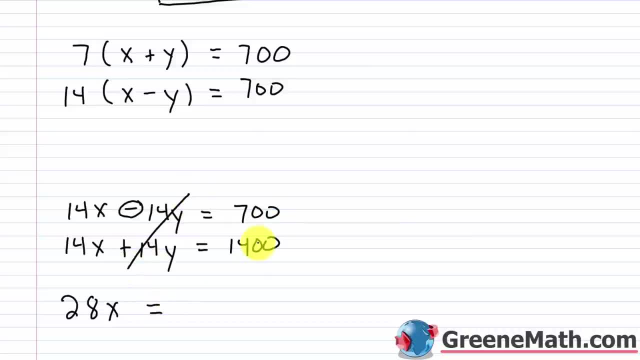 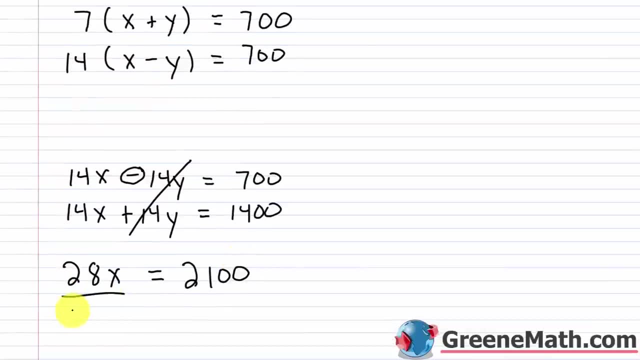 that's gonna be eliminated, And then this equals 700 plus 1400, which is 2100 or 2100.. So now to get X by itself, I divide both sides of the equation by 28.. And that's gonna give me that X is equal to 75. 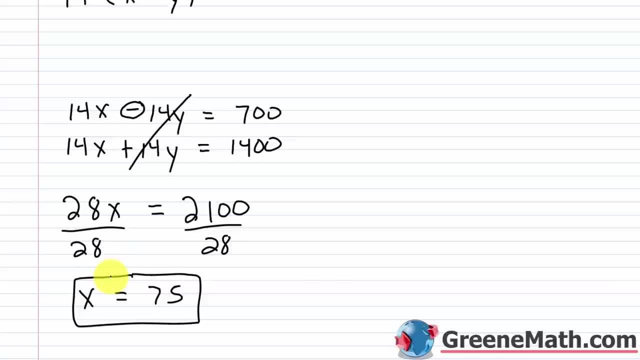 But again, I'm not done. I've gotta find out the value for Y. So let's go back and look at one of these original equations Again. we found that X was equal to 75.. So let's go back and look at one of these original equations Again. we found that X was equal to 75.. 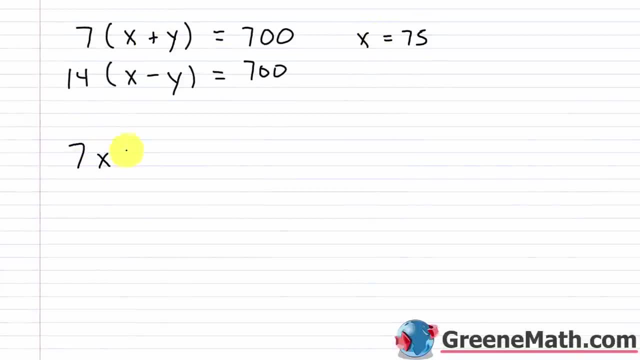 So let's go back and look at one of these original equations Again. we found that X was equal to 75.. So we had seven X plus seven Y, equals 700.. And we had 14 X minus 14 Y, equals 700. 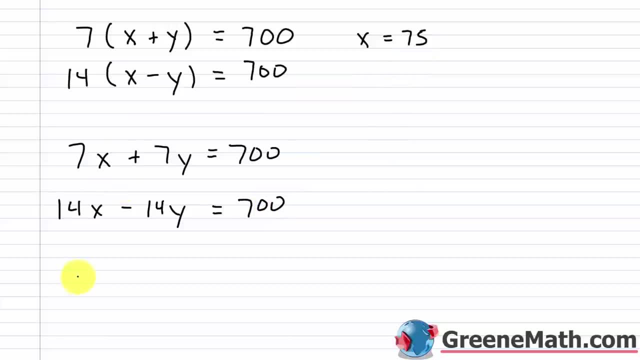 So plug in a 75 for X in either one. So let's just take the first one. So seven times 75 plus seven Y equals 700.. What's seven times 75? That's gonna be 525.. So we'd have 525 plus seven Y equals 700.. 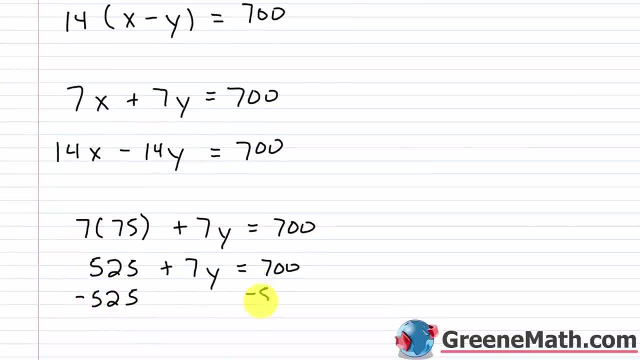 And then we'd subtract 525.. And then we'd subtract 525.. And then we'd subtract 525 from each side of the equation. That's gonna cancel, And we'd have seven. Y is equal to 700, minus 525 is 175. 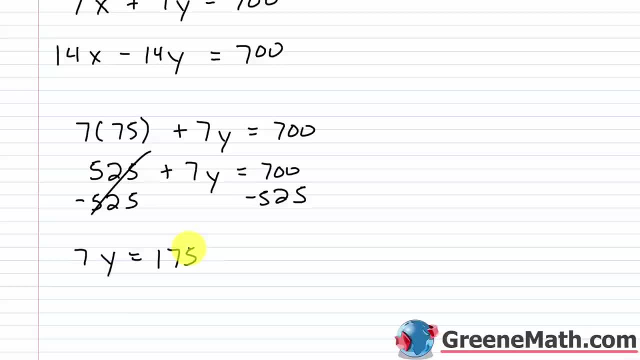 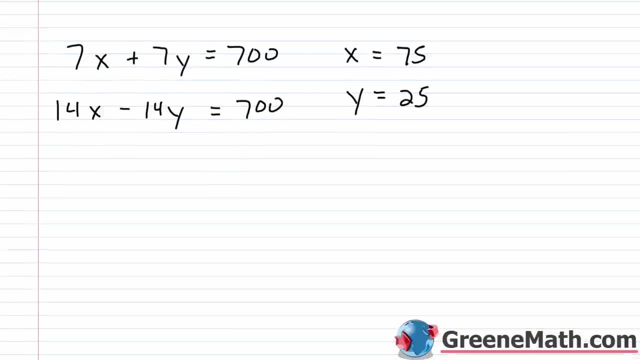 And we'd have seven. Y is equal to 700 minus 525 is 175.. And if I divide both sides of the equation by seven, I'm gonna end up with Y is equal to 25.. All right, so now we can write this as an ordered pair. 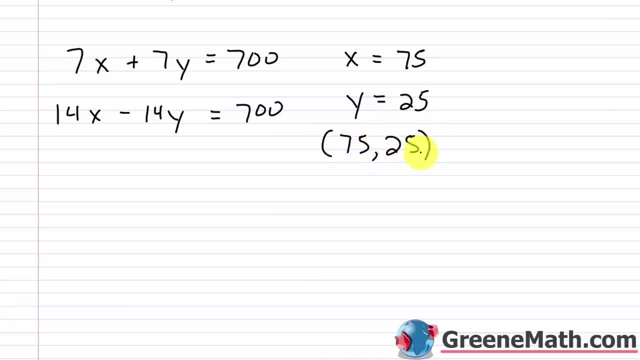 We'll say it's 75 comma 25.. And let's just check this guy in both equations, So we'd have seven times 75.. And let's just check this guy in both equations: times 75 plus 7 times 25 equals 700.. So 7 times 75 is 525.. Plus 7 times 25, that's 175.. 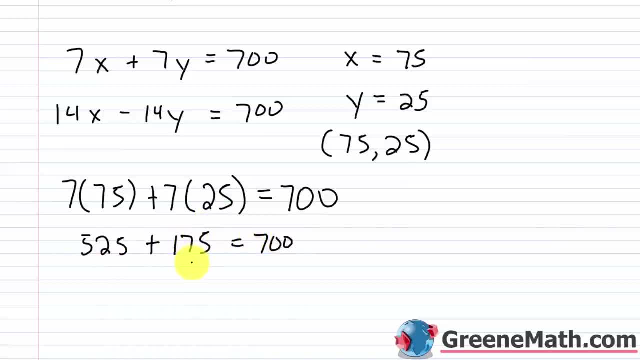 This should equal 700. And it does. 525 plus 175 is 700.. So these two sides are equal. So this one checks out. Then for the next one, we have 14 times 75 minus 14 times 25.. 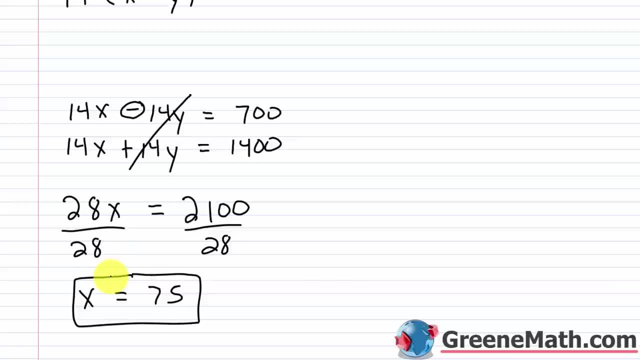 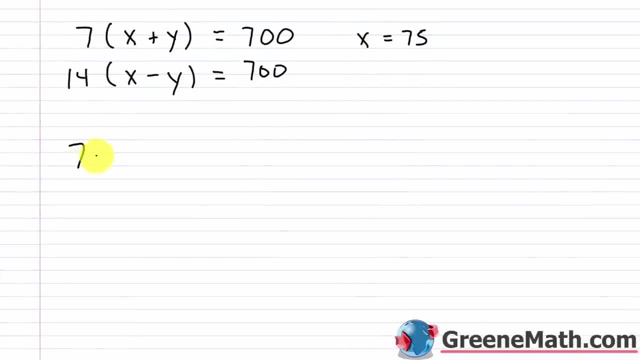 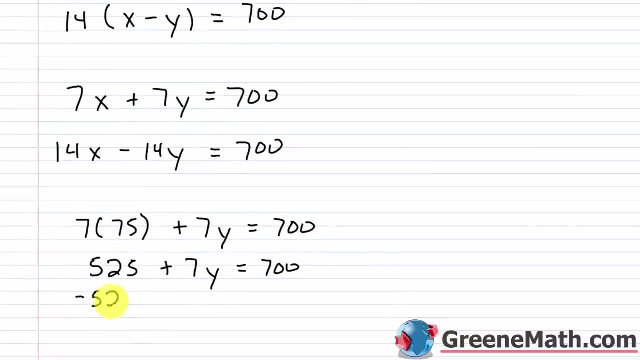 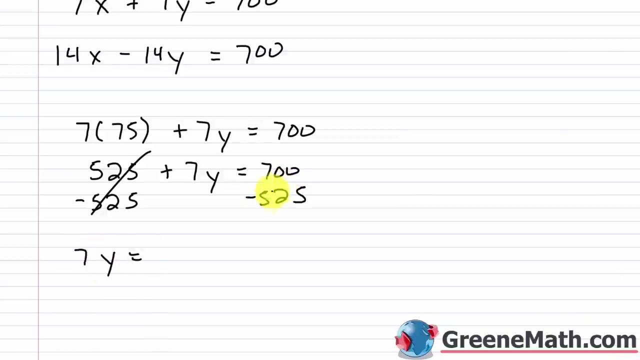 But again, I'm not done. I've got to find out the value for Y. So I'm going to go back and look at one of these original equations. Again, we found that X was equal to 75. So we had 7 X plus 7 Y equals 700. And we had 14 X minus 14 Y equals 700. So plug in a 75 for X in either one. So let's just take the first one. So 7 times 75 plus 7 Y equals 700. What's 7 times 75? That's going to be 525. So we'd have 525. Plus 7 Y equals 700. And then we'd subtract 525 away from each side of the equation. That's going to cancel. And we'd have 7 Y is equal to 700 minus 525 is 175. Then if I divide both sides of the equation by 7, I'm going to end up with Y is equal to 25. 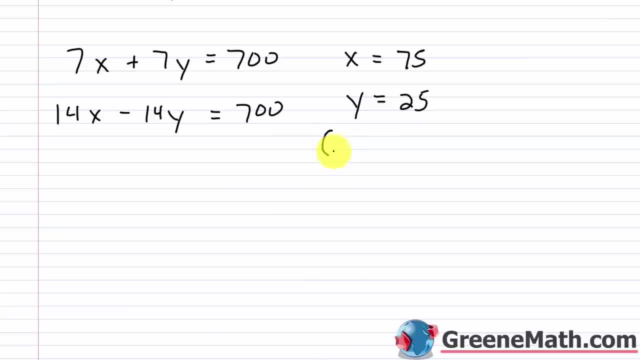 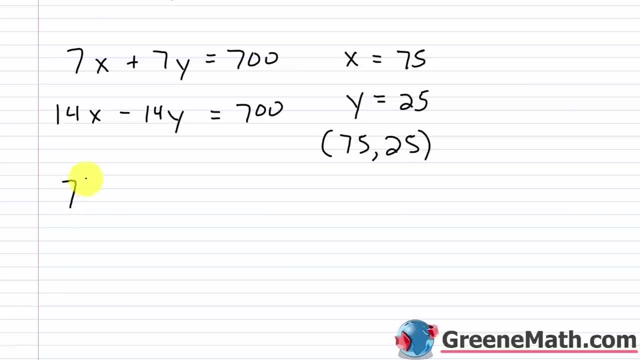 And both equations. So we'd have 7 times 75 plus 7 times 25 equals 700. So 7 times 75 is 525. Plus 7 times 25, that's 175. This should equal 700. And it does. 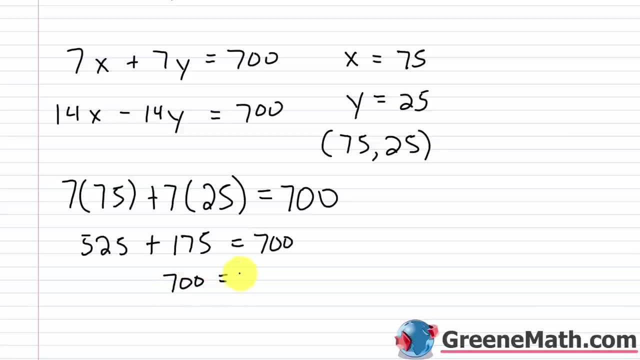 525 plus 175 is 700. So these two sides are equal. So this one checks out. 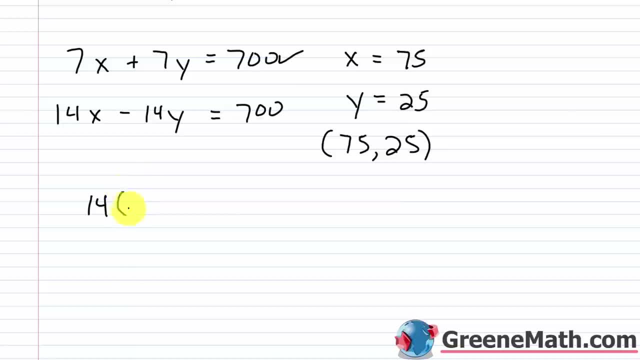 Then for the next one we have 14 times 75 minus 14 times 25 and this should equal 700. So 14 times 75 is 1,050 minus 14 times 25 which is 350 and this should equal 700 and again it does. 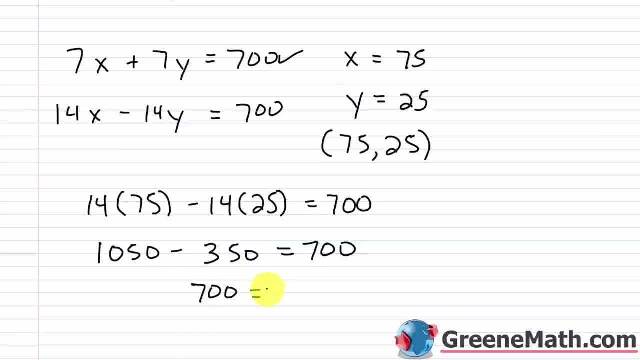 1,050 minus 350 is 700 so you get 700 equals 700 so it works out there as well. 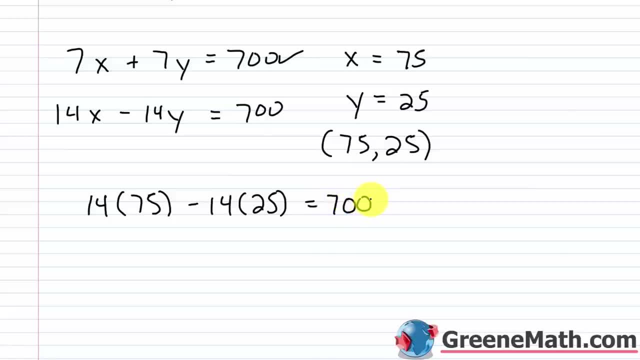 And this should equal 700.. So 14 times 75 is 1050.. Minus 14 times 25, which is 350. And this should equal 700. And again it does: 1050 minus 350 is 700. So you get 700 equals 700. So it works out there. 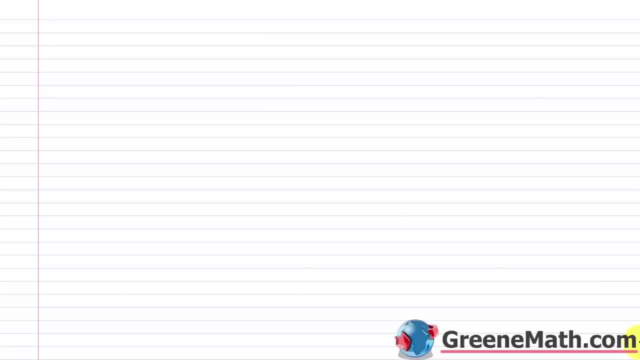 As well. All right, So remember, with the word problem, you always want to make a nice little sentence. So we're just going to say that the speed, the speed of the plane in still air, was 75 miles per hour And the wind speed, the wind speed. 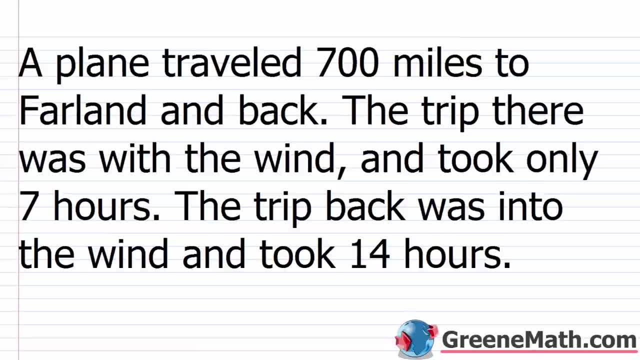 was 25 miles per hour. Let's see if this just makes sense in terms of what the problem said. So a plane traveled 700 miles to Farland and back. The trip there was with the wind and took only seven hours. So we know that if the plane was going 75 miles per hour and there was a 25 mile, 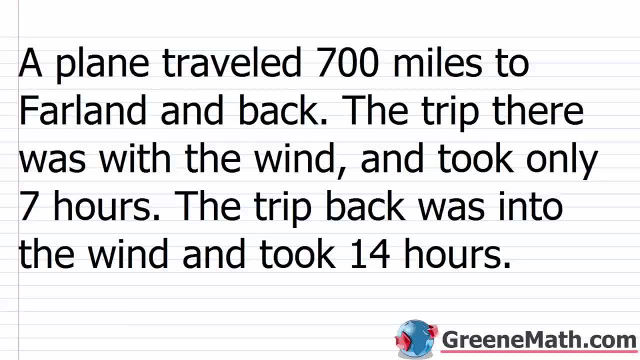 per hour wind, then each hour the plane is traveling 100 miles. So then it does this for seven hours, It's going to get 700 miles per hour, And then it does this for seven hours. And then it does this for seven hours, It's going to get 700 miles per hour, And then it does this for seven. 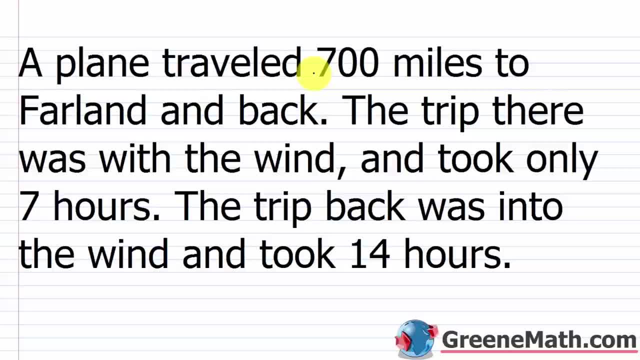 hours, It's going to get 700 miles worth of distance. So that checks out. Now, the trip back was into the wind. So if it's going 75 miles per hour and the wind is 25 miles per hour, you subtract, you would get 50 miles per hour. And then it does that for 14 hours. Well, 50 times 14. 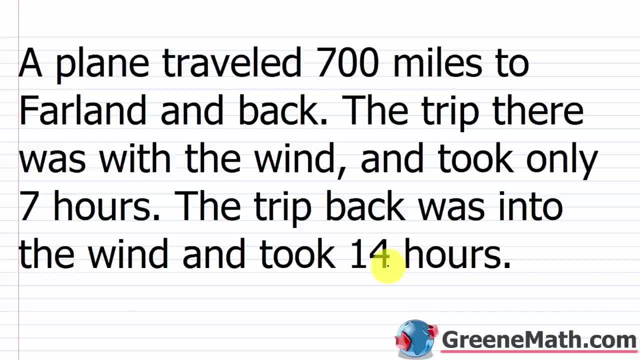 is also 700. So that checks out as well. So again, the speed of the plane in still air is 75 miles per hour And the wind speed is 25 miles per hour. Hello and welcome to Algebra. 1 Less Than 25.. 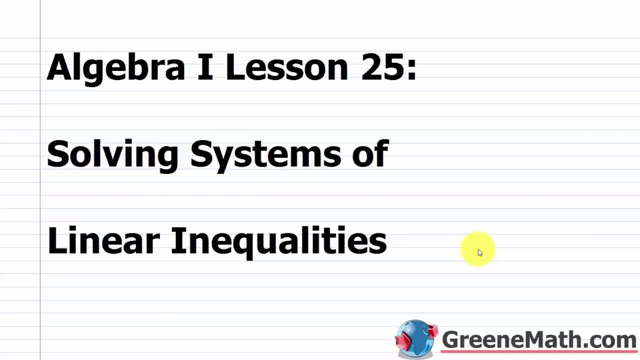 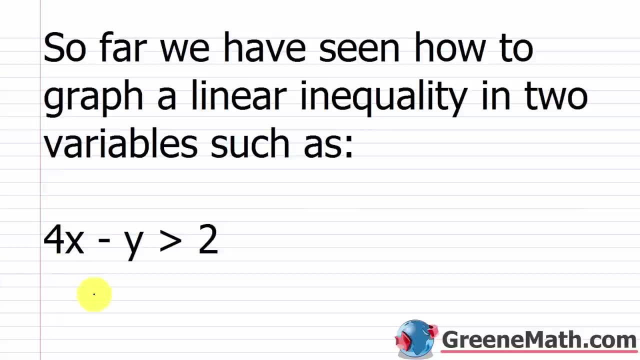 In this video we're going to learn about solving systems of linear inequalities. So so far we've seen how to graph a linear inequality in two variables such as- and I have a quick example for us: we have 4x minus y is greater than two. Now there's a few different methods. 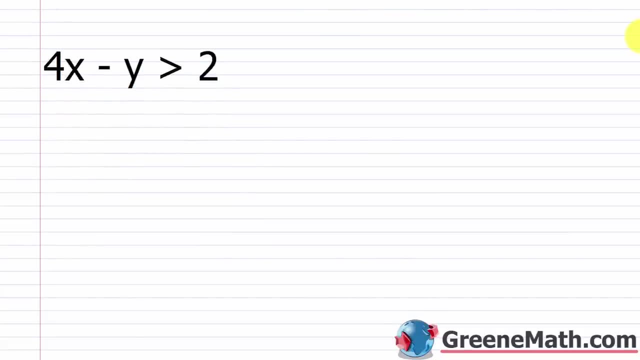 to kind of graph this, but the quickest one for me is to solve this for y. So in other words, I would subtract 4x away from both sides of the inequality, I would have negative y and I would subtract 4x away from both sides of the inequality. So in other words, 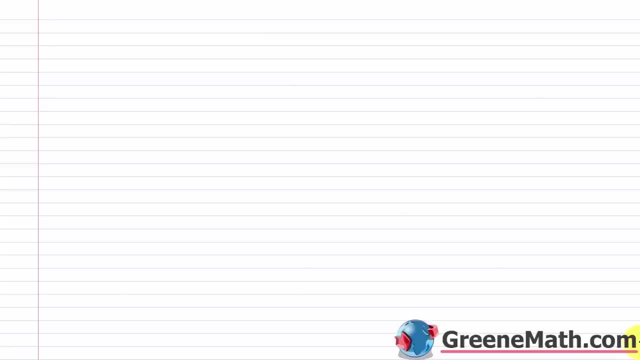 Alright so remember with the word problem you always want to make a nice little sentence. So we're just going to say that the speed, the speed of the plane in still air was 75 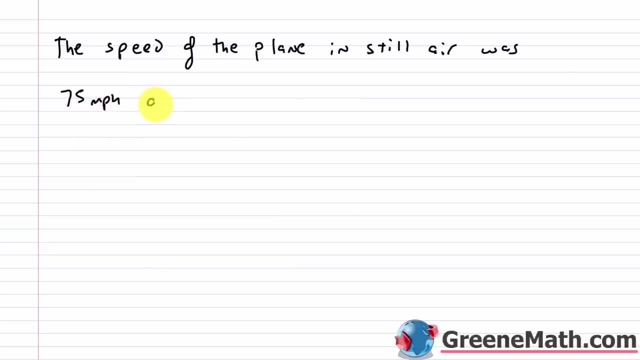 miles per hour and the wind speed, the wind speed was 25 miles per hour. Now let's see if this just makes sense in terms of what the problem said. 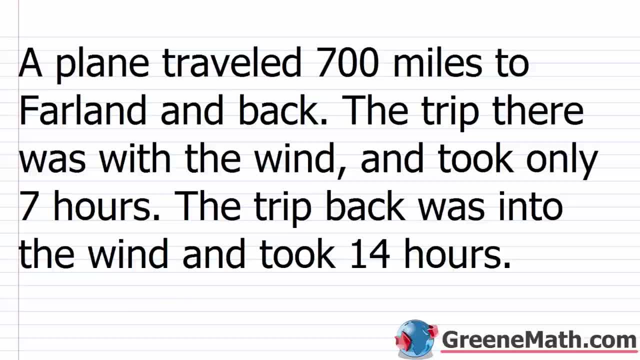 So a plane traveled 700 miles to Far Allen and back. 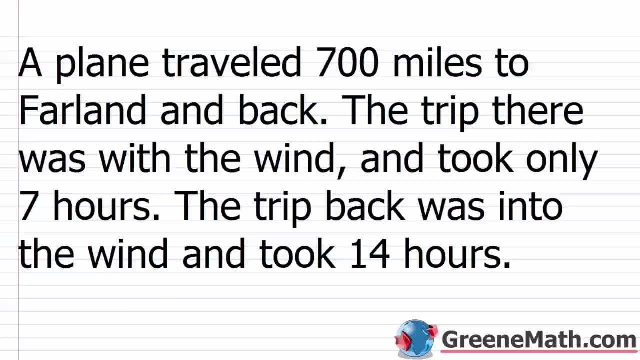 The trip there was with the wind and took only 7 hours. So we know that if the plane was going 75 miles per hour and there was a 25 mile per hour wind then each hour the plane is traveling 100 miles. So then it does this for 7 hours. It's going to get 700 miles worth of distance. 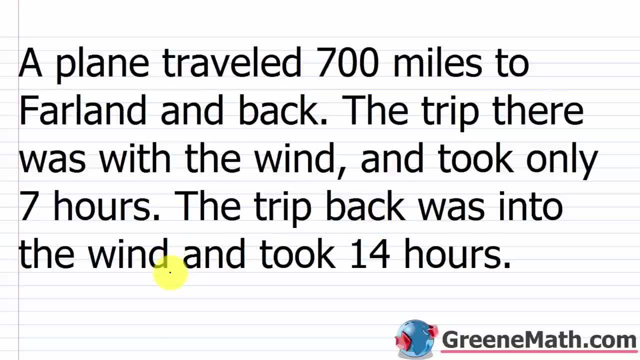 So that checks out. Now the trip back was into the wind. 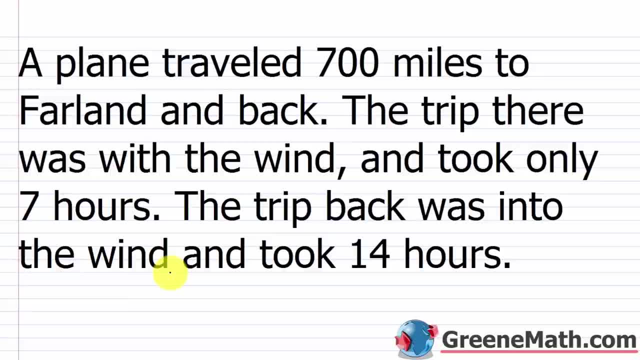 So if it's going 75 miles per hour and the wind is 25 miles per hour you subtract you would get 50 miles per hour and then it does that for 14 hours. 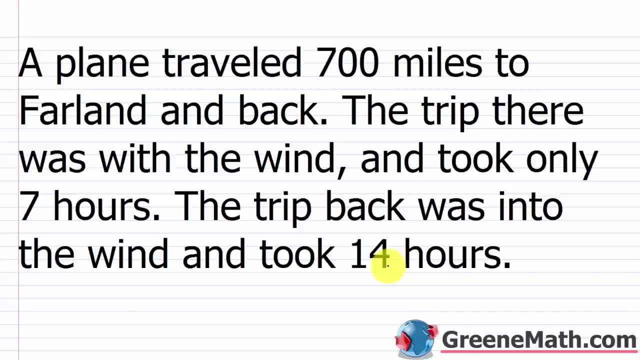 Well 50 times 14 is also 700. So that checks out as well. 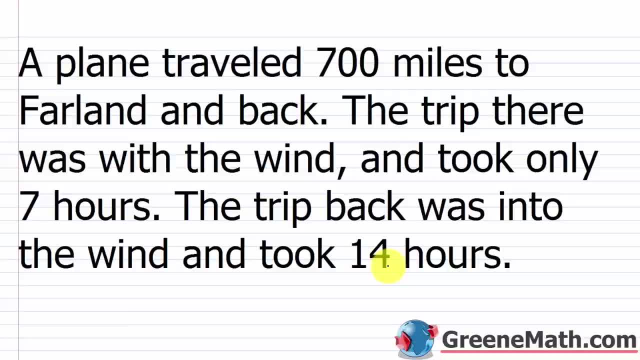 So again the speed of the plane in still air is 75 miles per hour and the wind speed is 25 miles per hour. 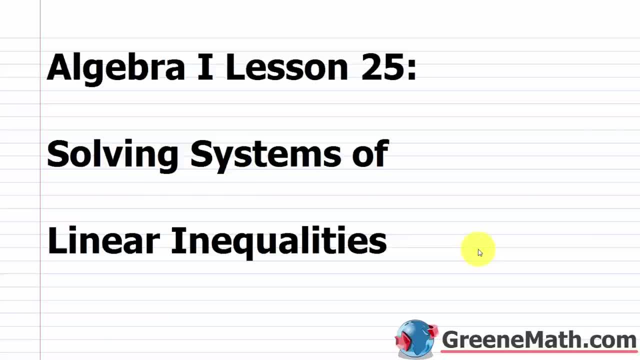 Hello and welcome to Algebra 1 Lesson 25. In this video we're going to learn about solving systems of less than 25 miles per hour. Let's get started. 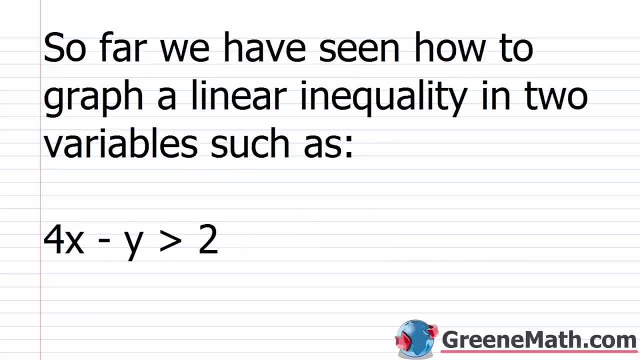 Let's start with the linear inequalities. So so far we've seen how to graph a linear inequality in two variables such as and I have a quick example for us. 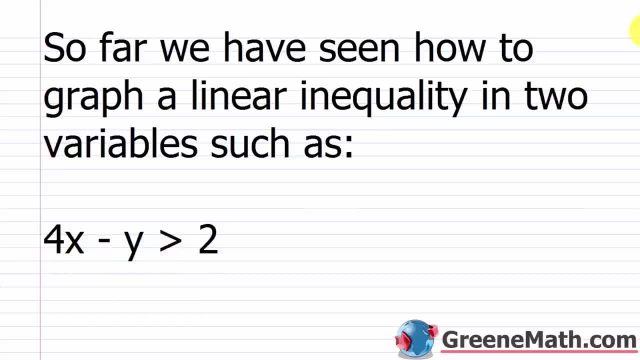 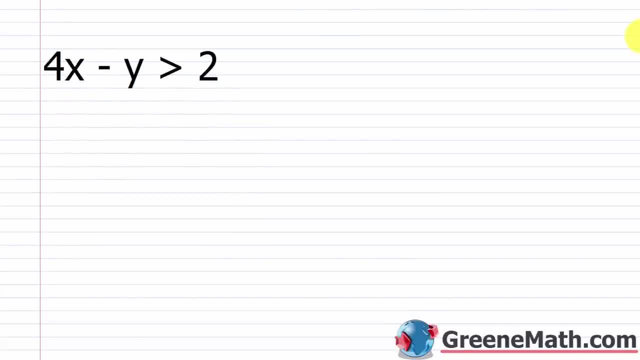 We have 4x minus y is greater than 2. Now there's a few different methods to kind of graph this but the quickest one for me is to solve this for y. So in other words I would subtract 4x away from both sides of the inequality. I would have negative y is greater than. Negative 4x plus 2. And then I would divide both sides of the inequality by negative 1. And remember if I'm dividing by a negative or I'm multiplying by a negative I've got to flip the direction of the inequality. 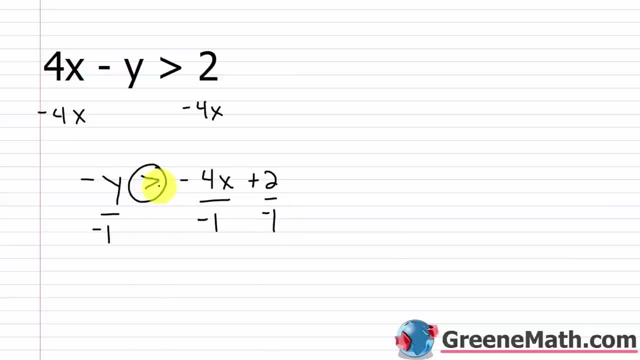 So this symbol right here tells me I have a greater than. I want to make this into a less than. So the direction of the inequality is going to change. Now negative y over negative 1 is y. So now it's y is less than. Negative 4 over negative 1 is positive 4. Then times x. And then 2 over negative 1 is negative 2. So I get y is less than 4x minus 2. 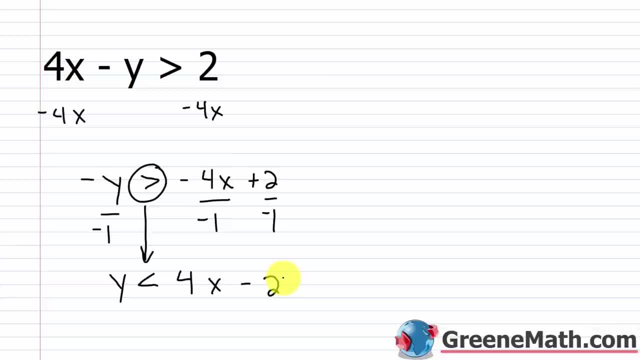 Now the reason I solve for y is it's easier for me to figure out where to shade. I don't have to go through and make a test point or anything like that. 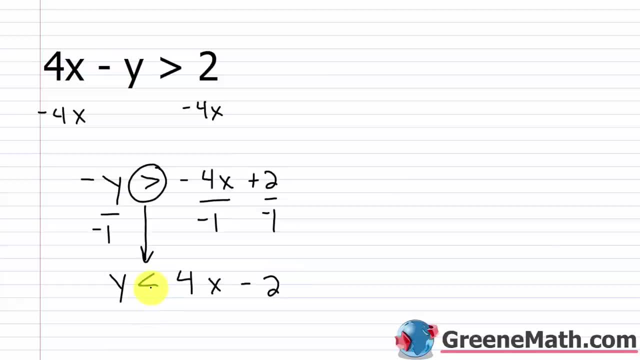 For a less than or a less than or equal to I just shade below the line. Now I'm getting ahead of myself. 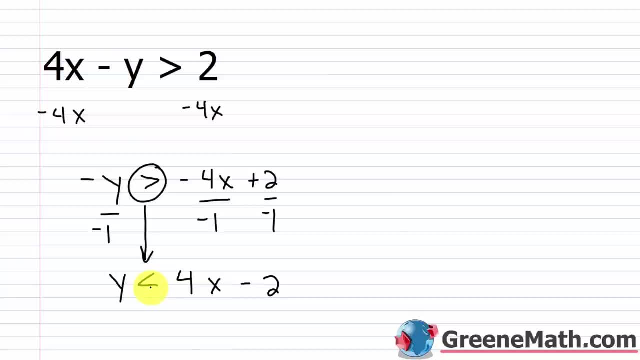 Remember this line that I'm talking about is called the boundary line. Okay. And we create the boundary line by replacing the inequality symbol with an equal symbol. 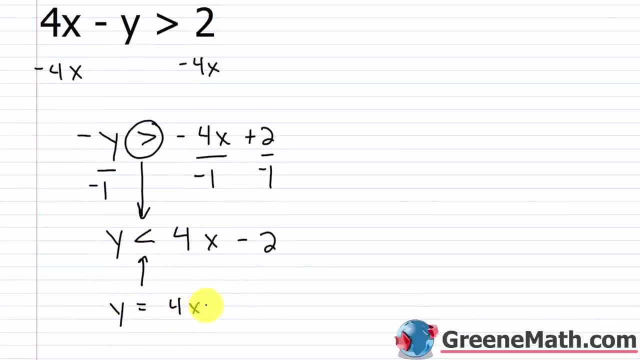 So I would graph y equals 4x minus 2 to begin. So let's go down to the coordinate plane. 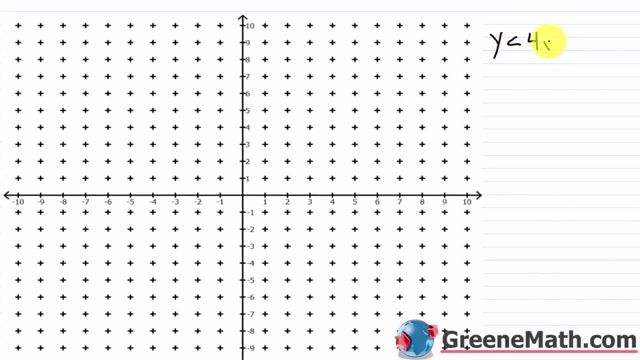 So again, we have y is less than 4x minus 2. And then our boundary line, we're going to graph y equals 4x minus 2. 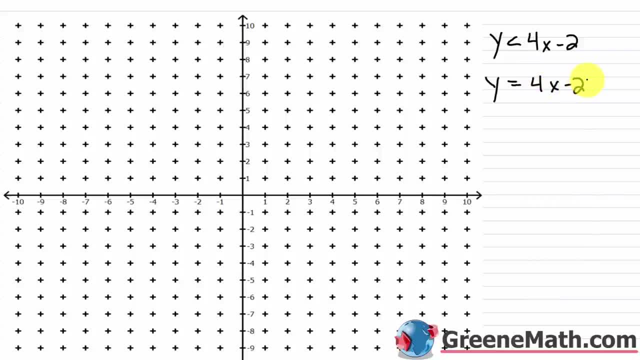 So one other piece of information before we kind of draw this boundary line. Remember, there's two different situations. 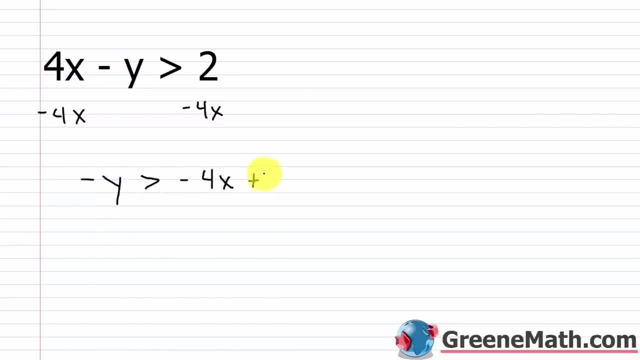 y is greater than negative 4x plus two. And then I would divide both sides of the inequality by negative one. And remember, if I'm dividing by a negative or multiplying by a negative, I've got to flip the direction of the inequality. So this symbol right here tells me I have a. 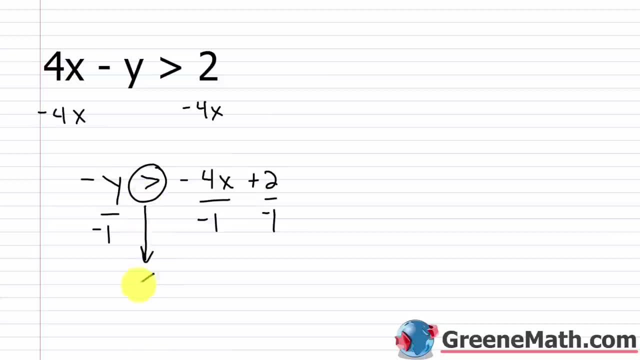 greater than I want to make this into a less than okay. so the direction of the inequality is going to change. Now negative y over negative, one is y, So now it's y is less than negative. four over negative, one is positive four and times x, and then two over negative. one is negative two. 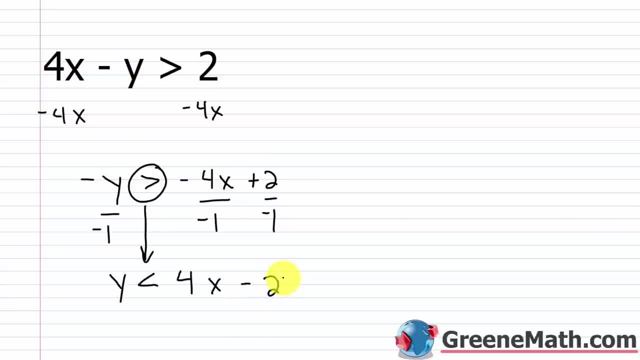 So I get: y is less than 4x minus two. Now the reason I solve for y is it's easier for me to figure out where to shade. I don't have to go through and make a test point or anything like that For a less than or less than or equal to. I just shade below the line. Now I'm getting ahead. of myself. Remember this line that I'm talking about. I'm going to shade below the line, So I'm going to shade below the line. So I'm going to shade below the line. So I'm going to shade below the line. 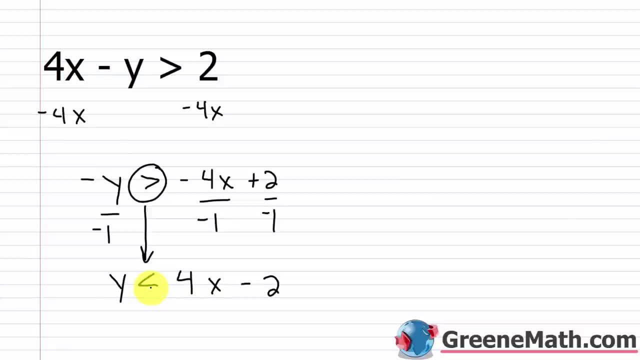 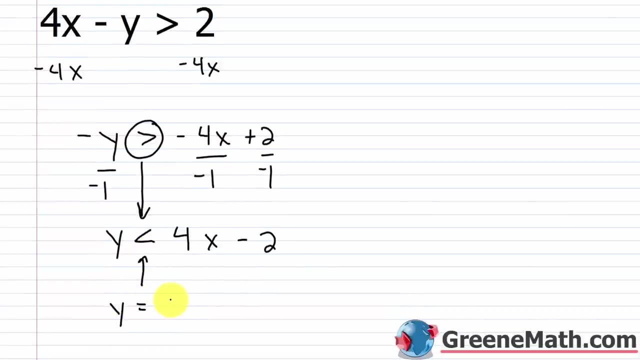 And I'm going to shade below the line. This is what I would call the boundary line, And we create the boundary line by replacing the inequality symbol with an equal symbol. So I would graph: y equals 4x minus two to begin. So let's go down to the coordinate plane. So again we have y is. 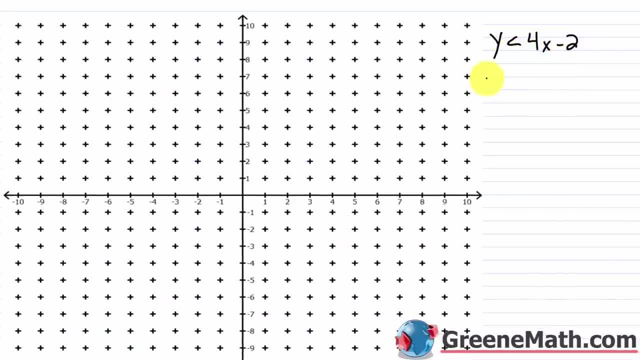 less than 4x minus two. And then our boundary line- we're going to graph y- equals 4x minus two. So one other piece of information before we kind of draw this boundary line. Remember there's two different situations. The boundary line will be a dashed line or a broken up line. 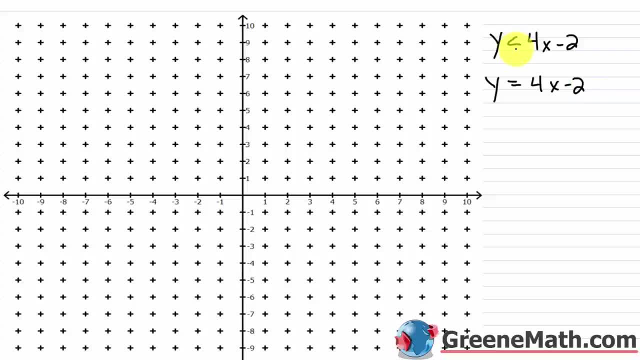 if you have a strict inequality like we have here In this case, the points that lie on the boundary line are not part of your solution. The other scenario that you'll run across is a non-strict inequality. So let's say I had a less than or equal to, or I had a greater than or equal to. 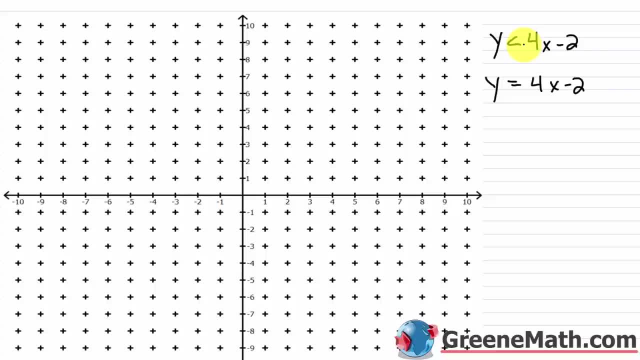 In this case, we want a solid boundary line, because the points on the line are part of the solution. For this specific case, though, we have a strict inequality, And so when we draw our boundary line, we want it to be dashed or broken up. 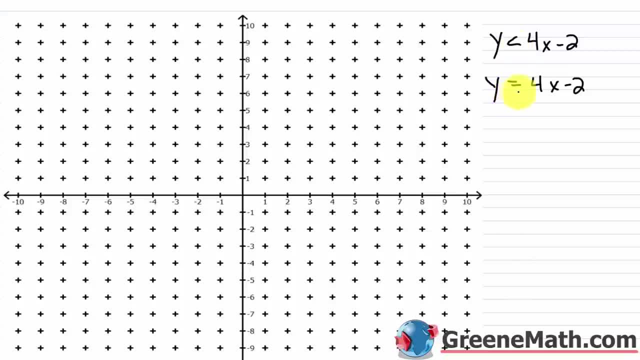 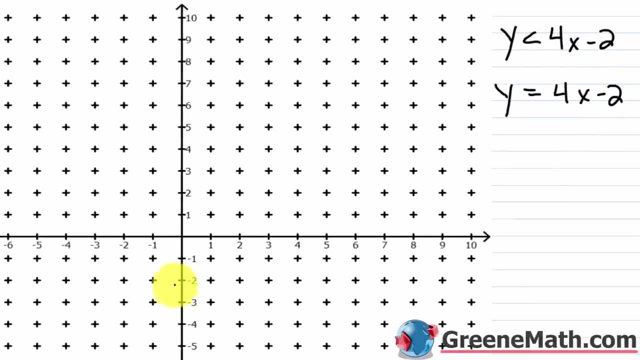 Again, all we need to do is graph the line. y equals 4x minus 2.. That's going to be our boundary line. So the y-intercept occurs at 0 comma negative 2.. So that's right here, And my slope is positive 4.. 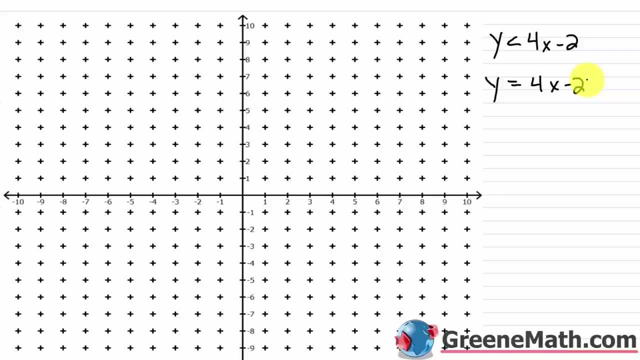 The boundary line will be a dashed line or a broken up line if you have a strict inequality like we have here. In this case, the points that lie on the boundary line are not part of your solution. The other scenario that you'll run across is a non-strict inequality. So let's say I had a less than or equal to or I had a greater than or equal to. In this case, we want a solid boundary line because the points on the line are part of the solution. 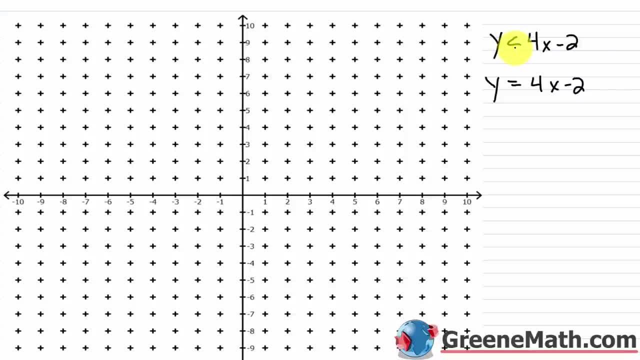 For this specific case, though, we have a strict inequality. And so when we draw our boundary line, we're going to have a non-strict inequality. 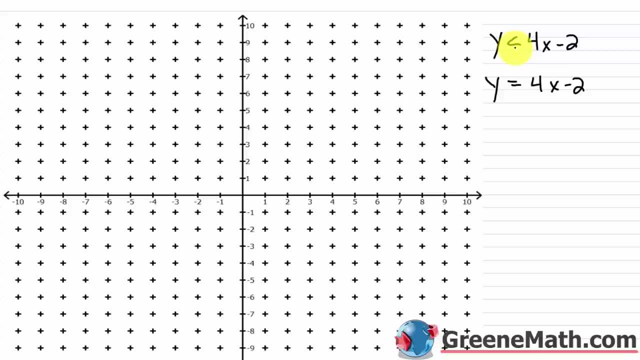 So when we draw our boundary line, we want it to be dashed or broken up. Again, all we need to do is graph the line y equals 4x minus 2. That's going to be our boundary line. 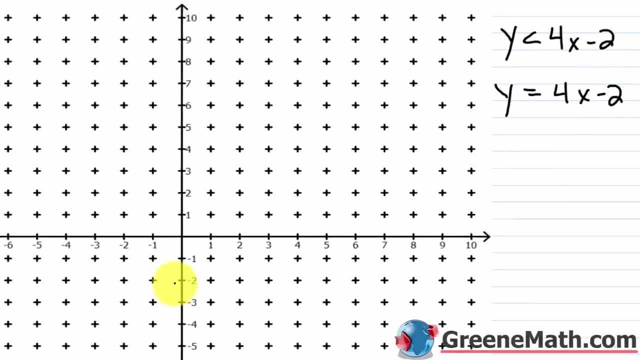 So the y-intercept occurs at 0 comma negative 2. So that's right here. And my slope is positive 4. So I'm going to go up 1, 2, 3, 4 to the right 1. 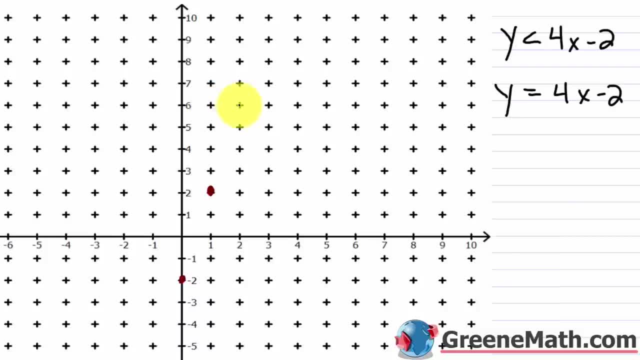 And I can do that one more time. Go up 1, 2, 3, 4 to the right 1. 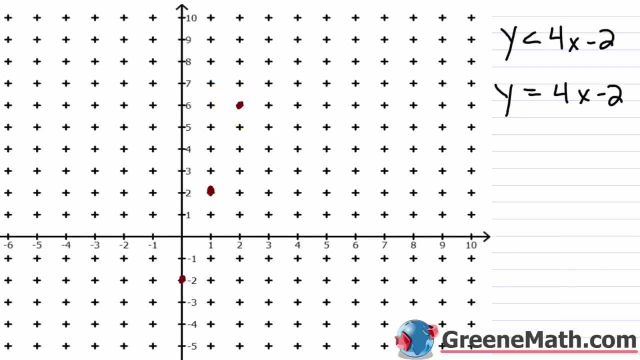 So let's draw a solid line. And then we'll use our eraser to kind of draw a line. And I'm going to break it up. 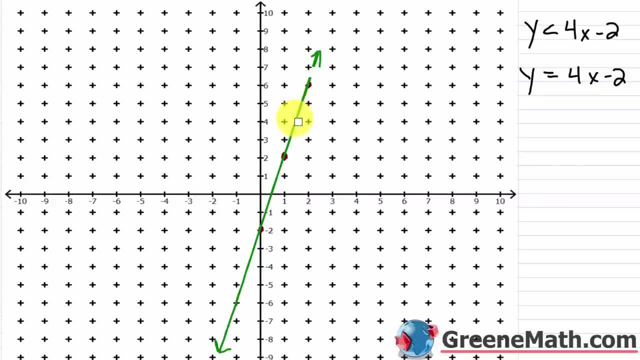 Okay, and I'm just going to take my eraser and just kind of break it up so that you know it's a dashed line. 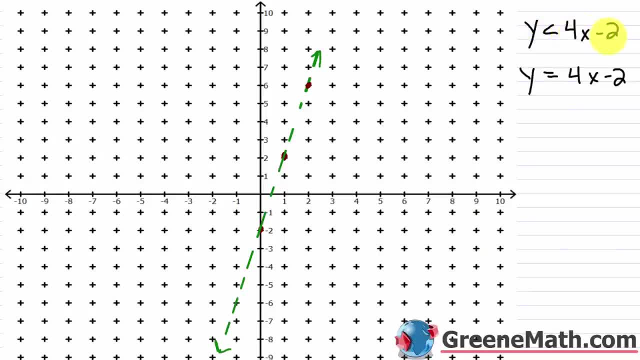 All right, so that's my boundary line for y is less than 4x minus 2. Now, one of the benefits to solving your inequality for y, if it's a less than or a less than or equal to, you just shade below the line. 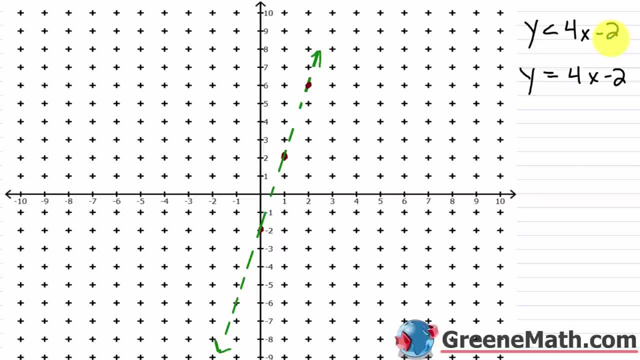 If it's a greater than or a greater than or equal to, you shade above the line. I know in your textbook, you probably read something about test points and all this other stuff. If you solved it for y, you don't need to do any of that stuff. 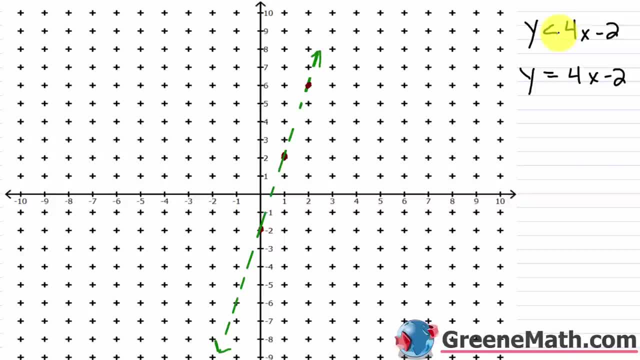 Again, less than or less than or equal to, shade below the line. Greater than or greater than or equal to, shade above the line. So this is a less than, so we shade below the line. Nice and simple. 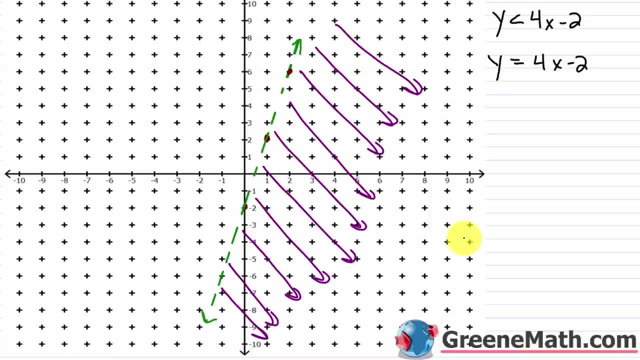 So basically, anything in that region would be a solution to our inequality, which was 4x minus y is greater than 2. 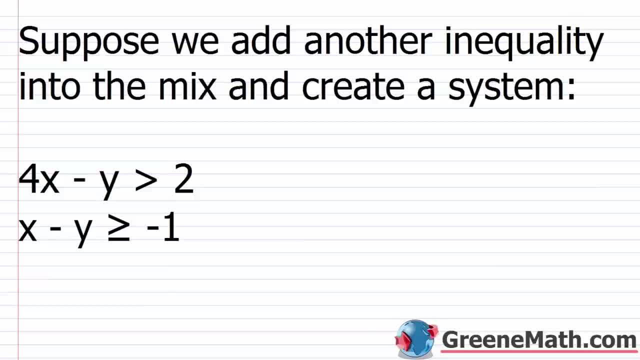 All right, so suppose we add another inequality into the mix and create a system. 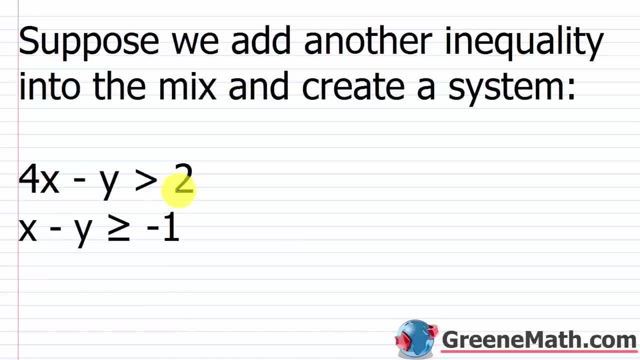 So this is the inequality we just graphed, 4x minus y is greater than 2. 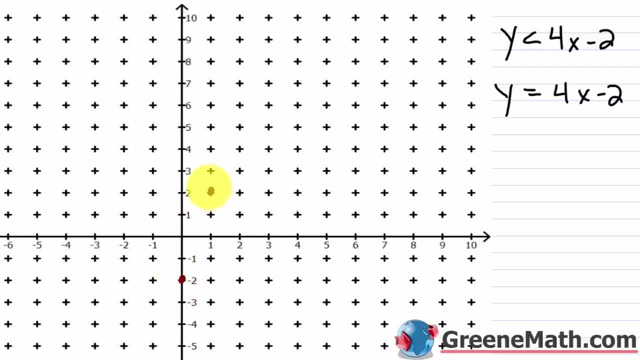 So I'm going to go up 1,, 2,, 3,, 4 to the right 1.. And I can do that one more time. Go up 1,, 2,, 3,, 4 to the right 1.. 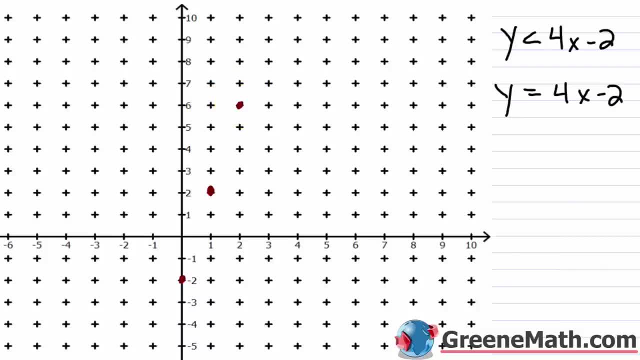 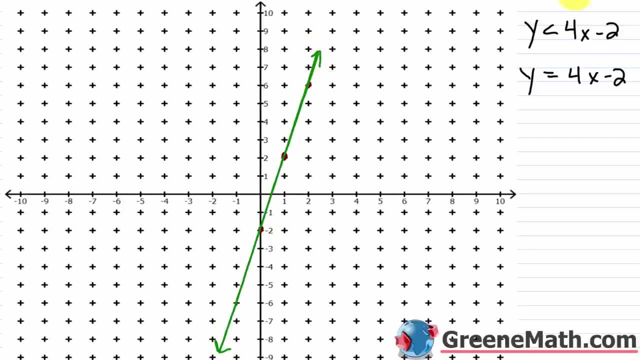 So let's draw a solid line and then we'll use our eraser to kind of break it up. Okay, and I'm just going to take my eraser and just kind of break it up, so that you know it's a dashed line. 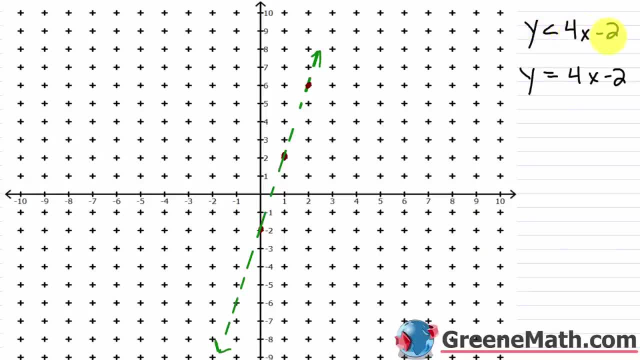 All right. so that's my boundary line, for y is less than 4x minus 2.. Now, one of the benefits to solving your inequality for y: if it's a less than or equal to or equal to 2, you just shade below the line. 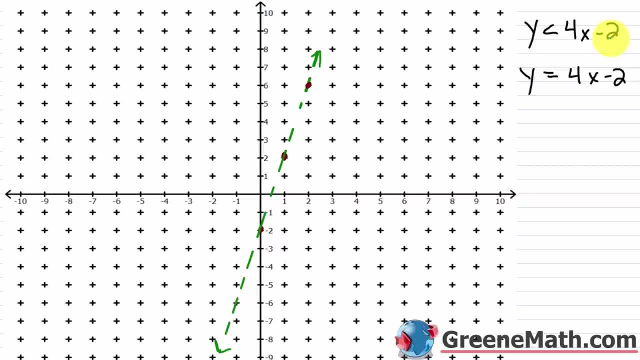 If it's a greater than or greater than or equal to you shade above the line. I know in your textbook you probably read something about test points and all this other stuff. If you solved it for y, you don't need to do any of that stuff. 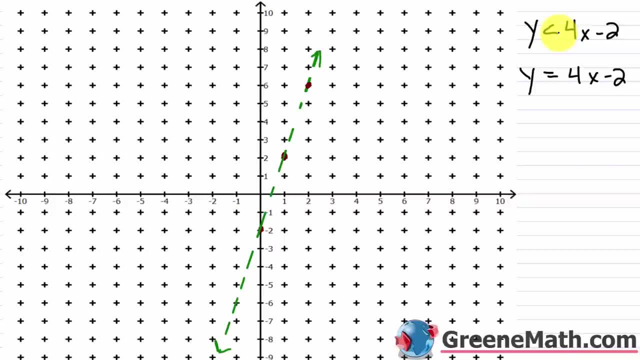 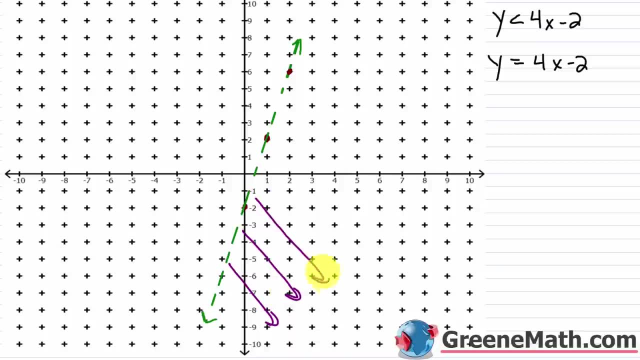 Again, less than or less than or equal to shade below the line. Greater than or greater than or equal to shade above the line. So this is a less than, so we shade below the line. Nice and simple. So basically, anything in that region would be a solution to our inequality. 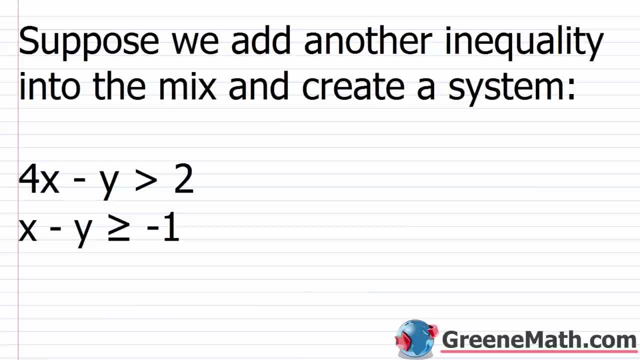 which was 4x minus y, is greater than 2.. All right, so suppose we add another inequality into the mix and create a system. So this is the inequality we just graphed: 4x minus y is greater than 2.. 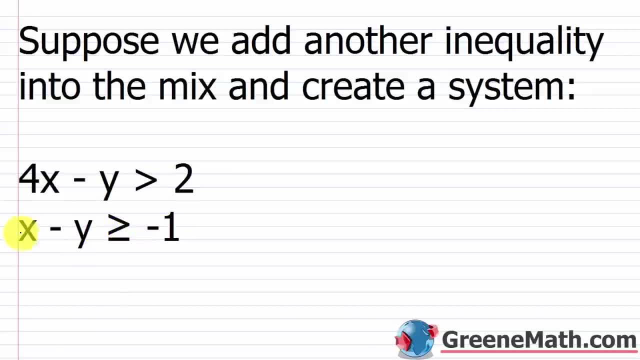 What about this one? x minus y is greater than or equal to negative 1? Well, let's graph this one real quick. I would solve it for y, so I'm just going to subtract x away from each of the two. I would divide both sides of the inequality by negative 1.. 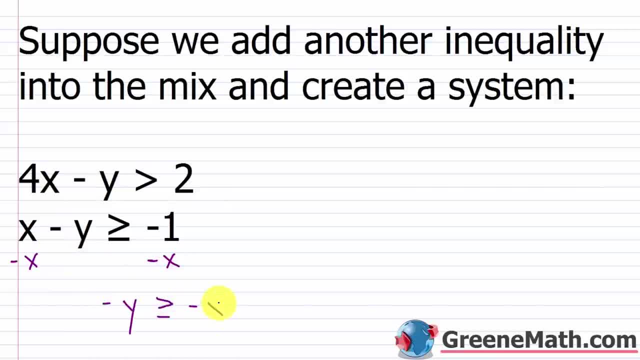 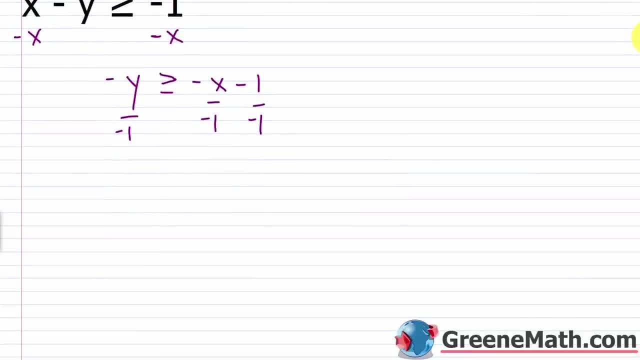 And I would have: negative y is greater than or equal to negative x minus 1.. I would divide both sides of the inequality by negative 1.. Scroll down, get a little rune going. So I would have y. this would flip. all right, I've got to flip the direction of the inequality. 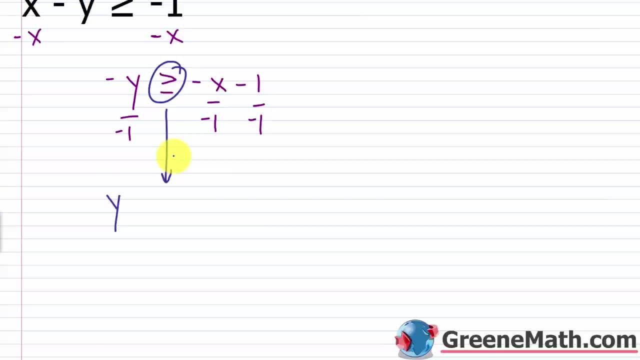 Right now it's a greater than or equal to. so I'm going to flip that direction and now it's going to be a less than or equal to, And then negative over negative is positive. So this is just going to be a less than or equal to. What about this one, x minus y is greater than or equal to negative 1? 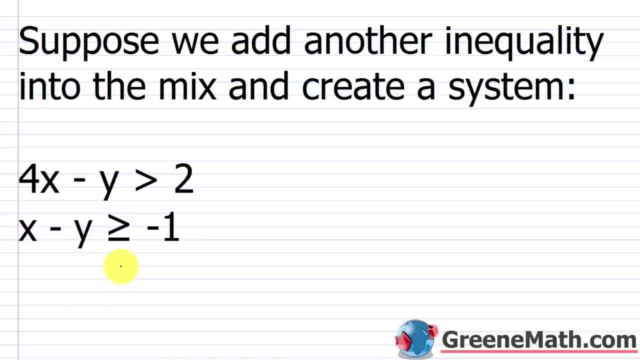 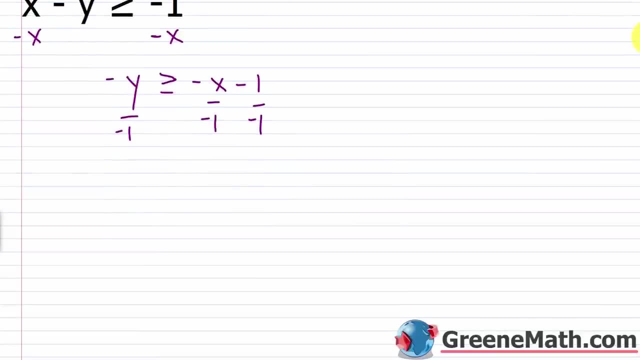 Well, let's graph this one real quick. I would solve it for y, so I'm just going to subtract x away from each side of the inequality. And I would have negative y. Y is greater than or equal to negative x minus 1. I would divide both sides of the inequality by negative 1. Scroll down, get a little rune going. 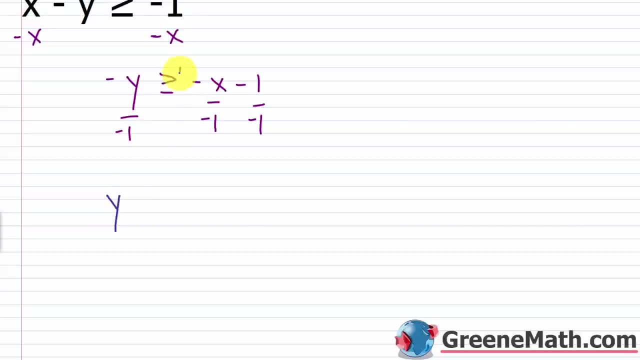 So I would have y. This would flip. All right, I've got to flip the direction of the inequality. Right now, it's a greater than or equal to. So I'm going to flip that direction. And now it's going to be a less than or equal to. And then negative over negative is positive. So this is just positive x. Negative over negative is positive. So plus 1. 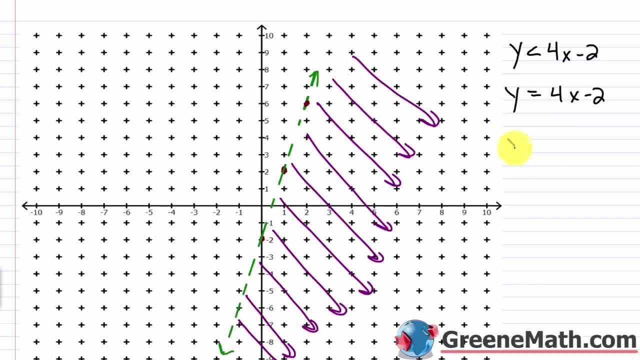 So y is less than or equal to x plus 1. So I'm looking at y is less than or equal to x plus 1. 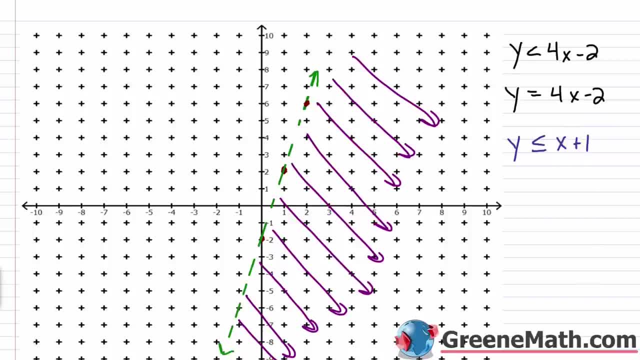 So again, I'm going to graph my boundary line to start. The boundary line is found by just replacing this inequality symbol with an equal symbol. 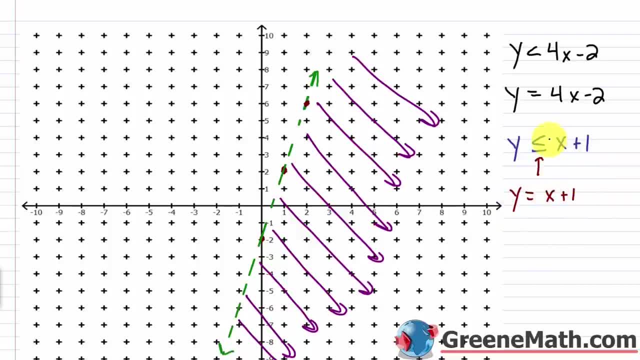 So I'm going to graph y equals x plus 1. And in this situation, we have a non-strict inequality. 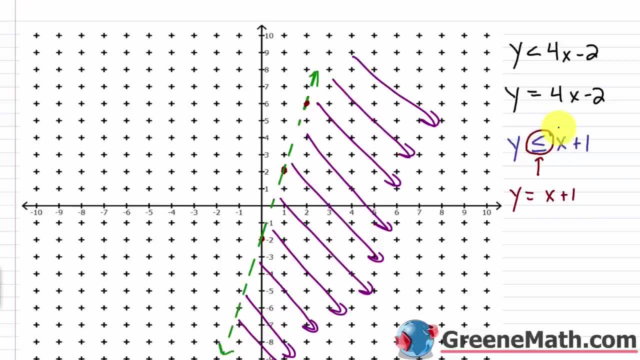 So we want our boundary line to be a solid line. So let's go ahead and graph this. So the y intercept will occur at 0. 0 comma 1. 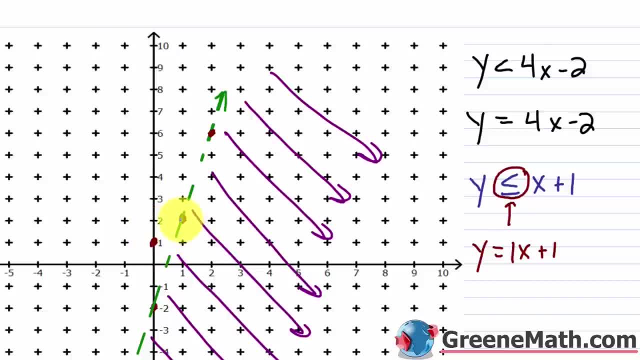 And then our slope is 1. So we go up 1 and to the right 1. So we share a point here. Up 1 and to the right 1. Up 1 and to the right 1. And so we have a few points going. 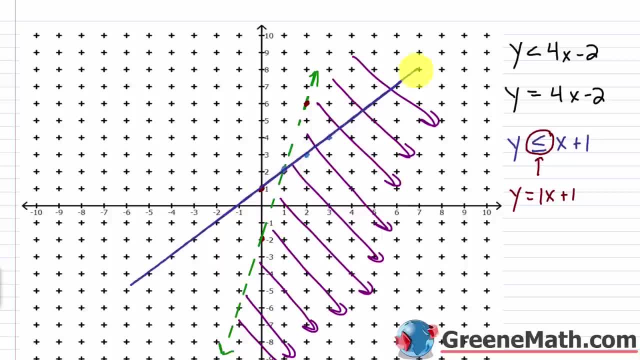 So let's go ahead and graph that guy. OK, remember, this is a solid line. So we're going to keep it that way. And then it's a less than or equal to. So that means I want to shade below the line. So let me use this kind of color. I'm going to use an orange. So I would shade everything that goes below this line. Now, I know there's a lot of stuff going on in the graph. It's kind of busy. 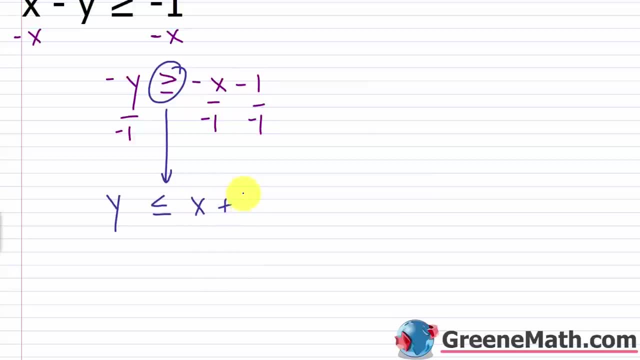 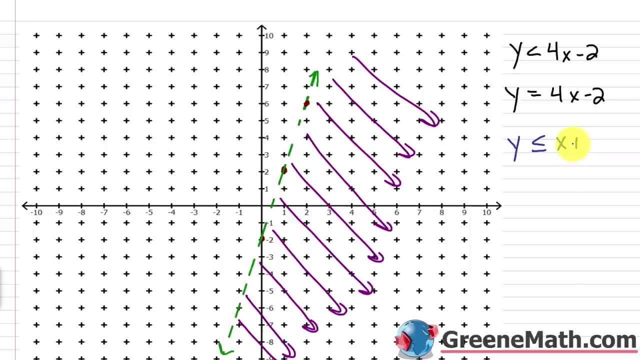 So this is just positive x negative over negative is positive, so plus 1.. So y is less than or equal to x plus 1.. So I'm looking at, y is less than or equal to x plus 1.. Now again, I'm going to graph my boundary line to start. 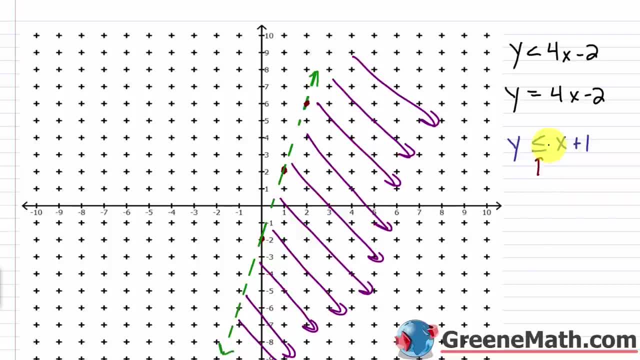 The boundary line is found by just replacing this inequality symbol with an equal symbol. So I'm going to graph: y equals x plus 1. And in this situation we have a non-strict inequality. So we want our boundary line to be a solid line. 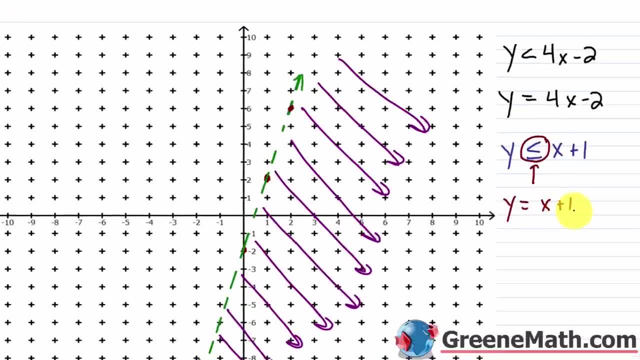 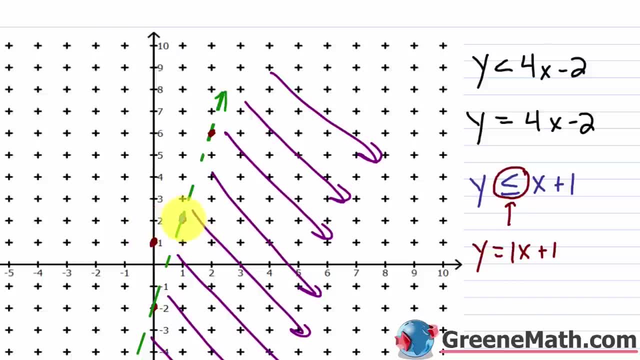 So let's do that, So let's go ahead and graph this. So the y-intercept would occur at 0 comma 1, so that's right there. And then our slope is 1, so we go up 1 and to the right, 1, so we share a point here. 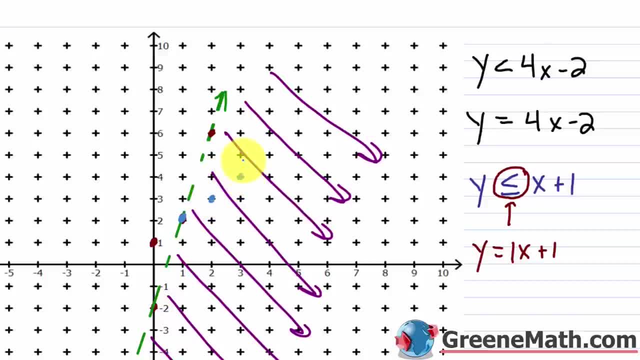 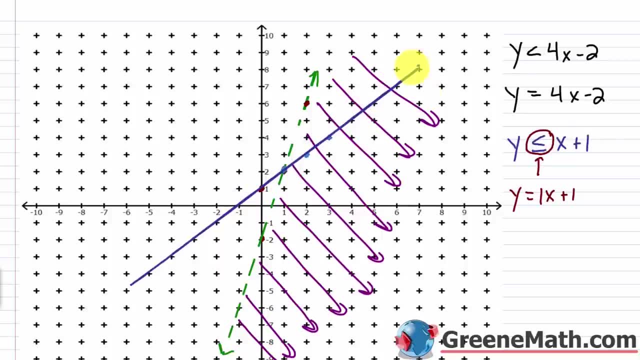 Up 1 and to the right 1,, up 1 and to the right 1, and so we have a few points going. So let's go ahead and graph that guy. Okay, remember, this is a solid line, so we're going to keep it that way. 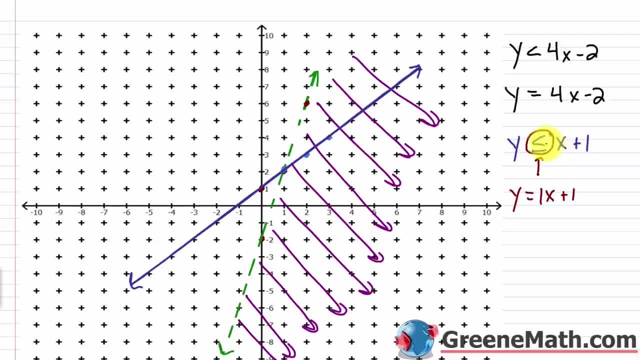 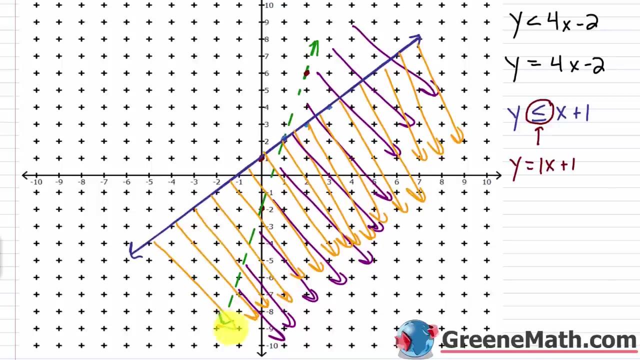 And then it's a less than or equal to, so that means I want to shade below the line, So let me use this kind of color. I'm going to use an orange, So I would shade everything that goes below this line. Now I know there's a lot of stuff going on in the graph. 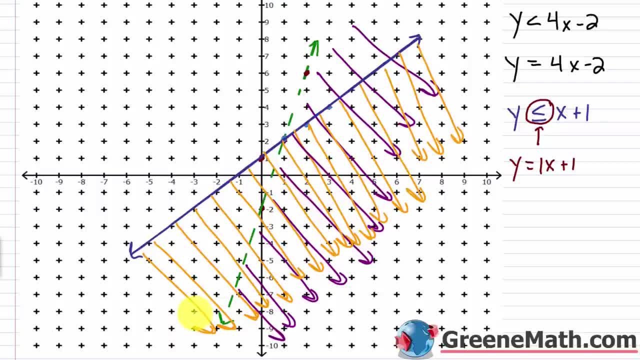 It's kind of busy. But what is the solution for the system? Well, recall that The solution for a system of linear equations is the single point that lies on both lines. So in this case, since we're dealing with inequalities, it's going to be the region of the coordinate plane where the two graphs are going to overlap. 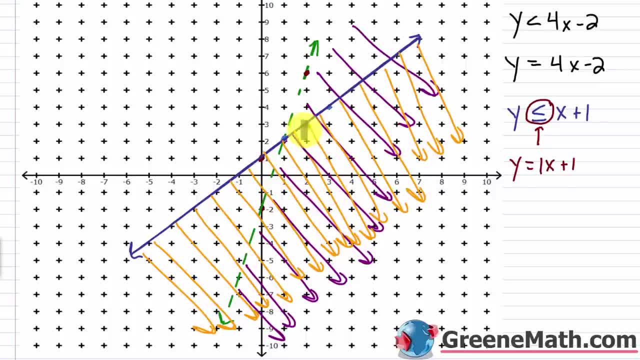 So if I take my highlighter here, where is that going to be? Well, it's got to be on this line, starting there- And I know I might have went over a little bit And then kind of following down this path here. 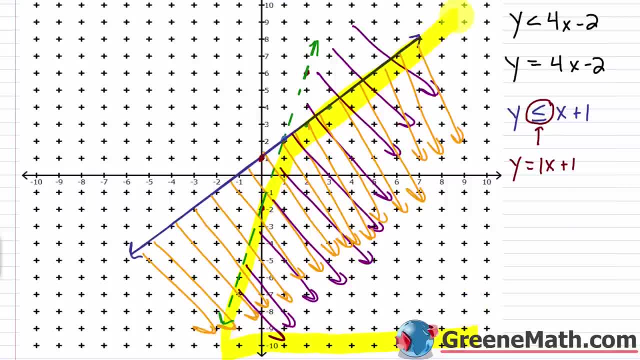 Kind of all this area, All this area, And it continues forever and ever and ever. But I'm just going to highlight the best that I can to kind of give you an idea here. Let me just kind of fill this in So you can see that. 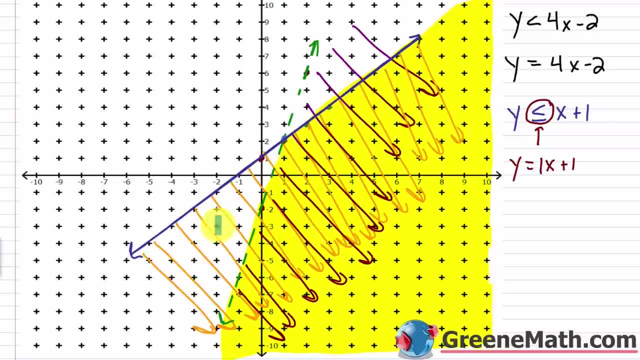 Let me kind of figure out a different color here. You can see that this part right here, this area right here, it satisfies one of them. So let me highlight this in blue: This satisfies one of them, but not both of them. 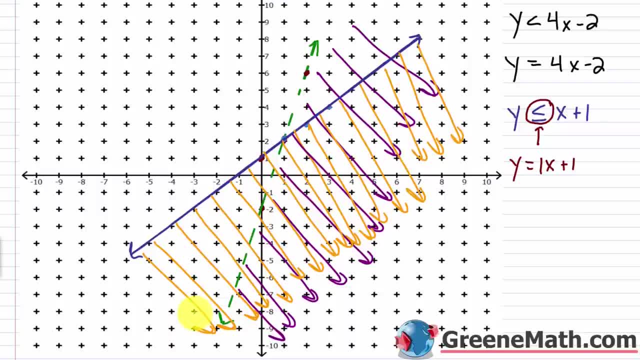 But what is the solution for the system? Well, recall that the solution for a system of linear equations is the single point that lies on both lines. So in this case, since we're dealing with inequalities, it's going to be the region of the coordinate plane where the two graphs are going to overlap. So if I take my highlighter here, where is that going to be? Well, it's got to be on this line starting there. 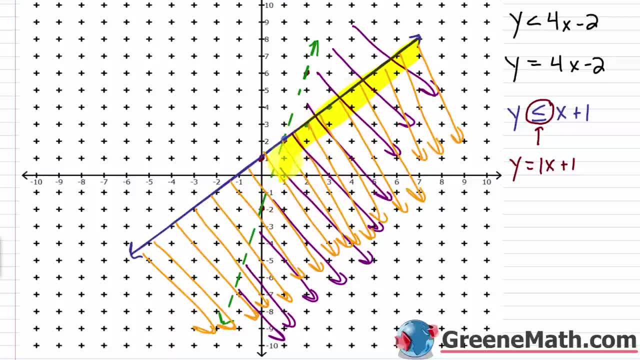 And I know I might have went over a little bit. And then kind of following down this path here. 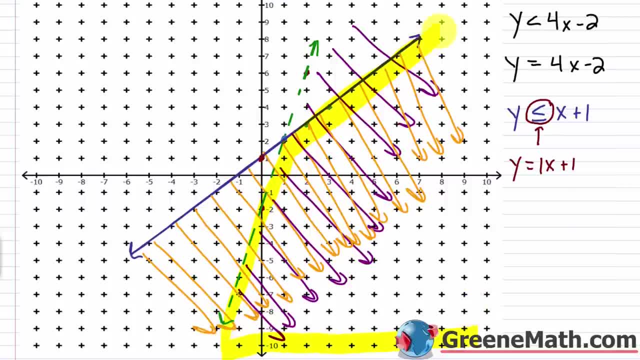 Kind of all this area. All this. This area. 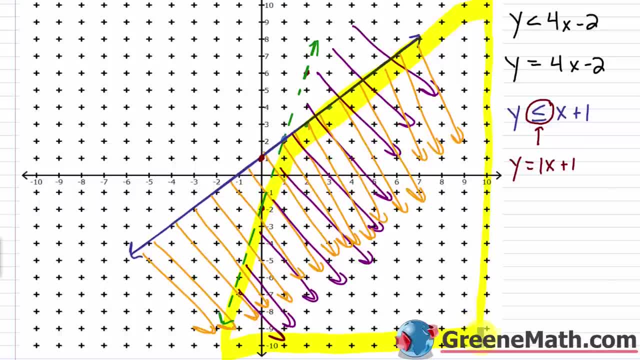 And it continues forever and ever and ever. But I'm just going to highlight the best that I can to kind of give you an idea here. Let me just kind of fill this in. So you can see that. Let me kind of figure out a different color here. 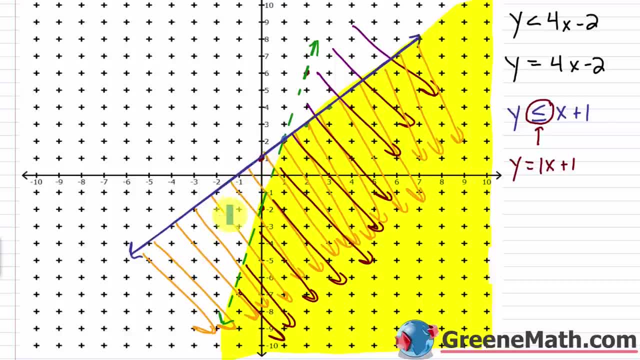 You can see that this part right here, this area right here, it satisfies one of them. So let me highlight this in blue. This satisfies one of them, but not both of them. So that's why it's not part of the solution. So let me go ahead and just erase all that. So this wouldn't be part of the solution. 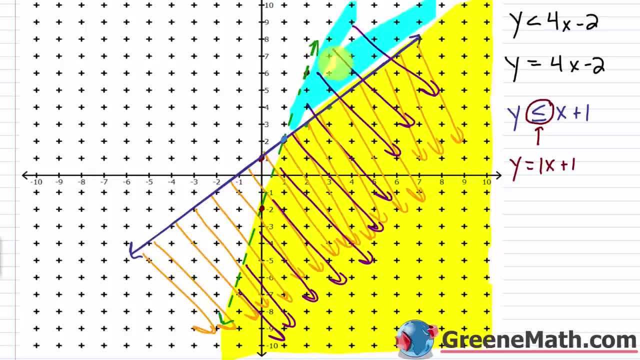 And this area up here is the same as well. This would satisfy one of them, but not both of them. So that's not part of the solution either. 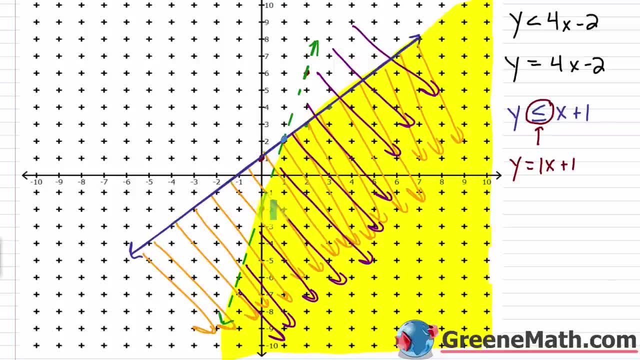 So I know I went over the line in some of the cases. But you can essentially see where the two graphs overlap. That's the part of the coordinate plane where y is less than 4x minus 2. And also y is less than or equal to x plus 1. So that specific area satisfies the system. All right. So pretty easy overall. Let's take a look at another one. 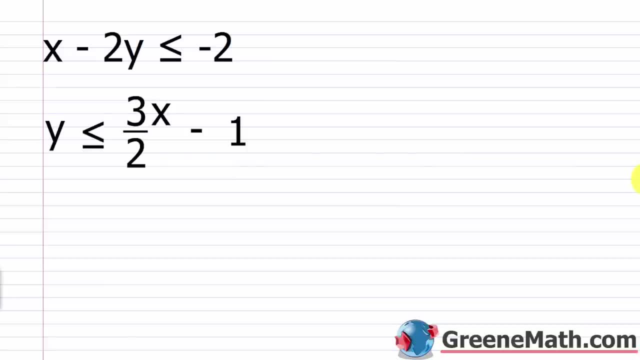 We have x minus 2y is less than or equal to negative 2. And we have y is less than or equal to 3 halves x minus 1. So this guy right here is already solved for y. So I don't need to do anything to that. I can just take it down and graph it. For this one, I want to solve it for y first. So let's pull this one down and do a little extra work to begin. 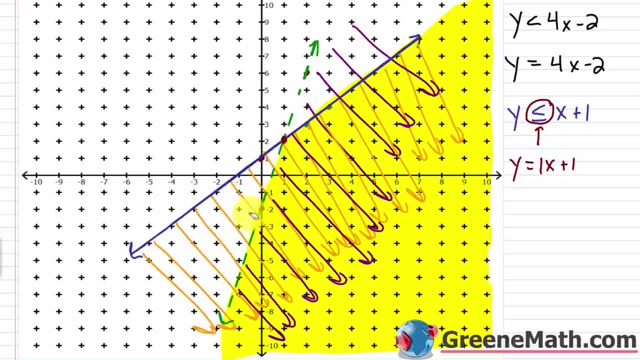 So that's why it's not part of the solution. So let me go ahead and just erase all that. So this wouldn't be part of the solution, And this area up here is the same as well. This would satisfy one of them, but not both of them. 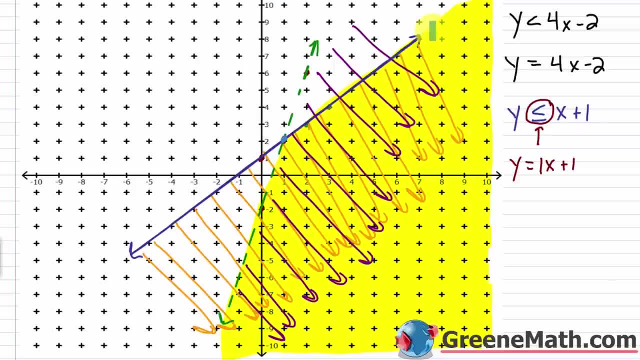 So that's not part of the solution either. So I know I went over the line in some of the cases, But you can essentially see where the two graphs overlap. That's the part of the coordinate plane where y is less than 4x minus 2.. 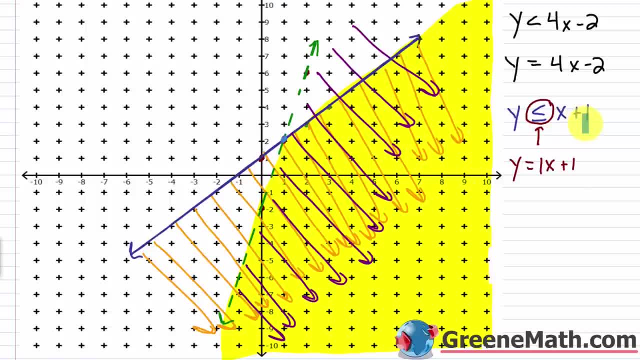 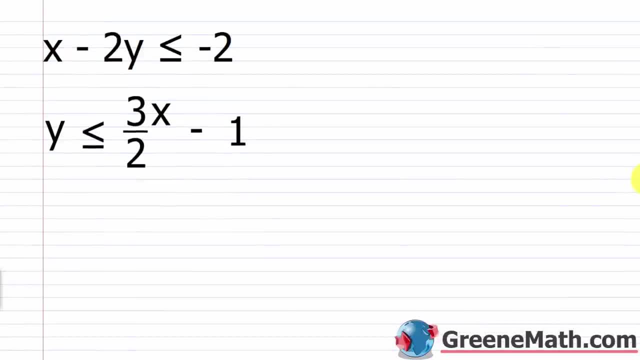 And also y is less than or equal to x plus 1.. So that specific area satisfies the system. All right, So pretty easy overall. Let's take a look at another one. We have x minus 2y is less than or equal to negative 2.. 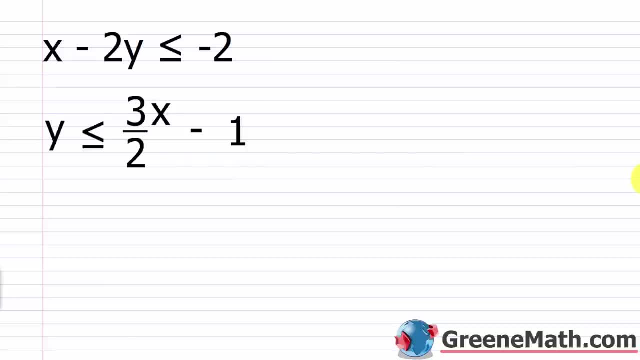 And we have: y is less than or equal to 3 halves x minus 1.. So this guy right here is already solved for y, So I don't need to do anything to that. I can just take it down and graph it For this one. I want to solve it for y first. 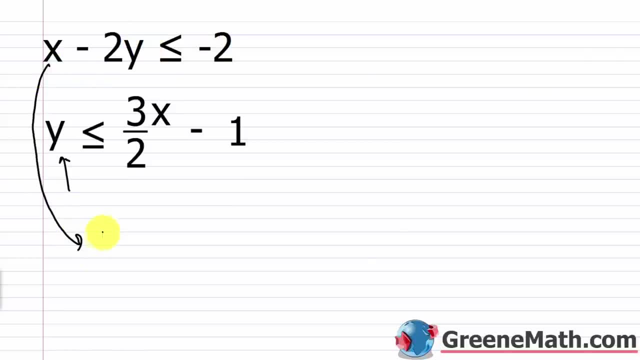 So let's pull this one down and do a little extra work. to begin, We have x minus 2y is less than or equal to negative 2.. So I would subtract x away from each side of the inequality And I'll have negative 2y is less than or equal to negative x minus 2.. 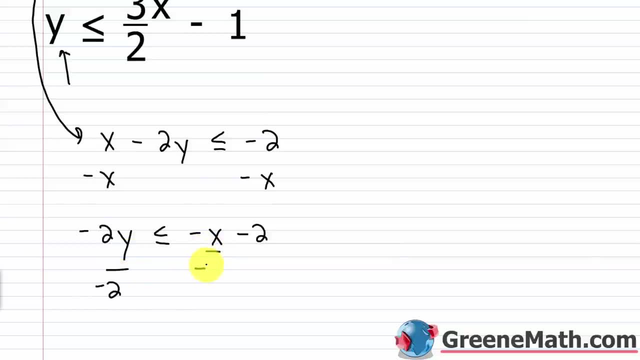 Now to get y by itself, I'm going to divide both sides of the inequality by negative 2.. So this guy is going to flip. Instead of it being a less than or equal to, it's going to become a greater than or equal to. 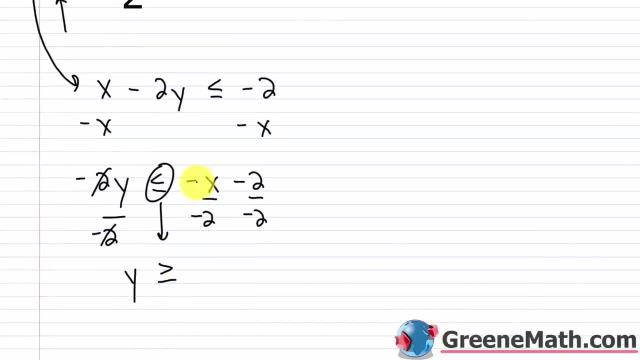 So this is going to cancel and become: y is greater than or equal to Negative over negative is positive. So this would be 1 half x, And then negative 2 over negative, 2 would be plus 1.. So I've got y is greater than or equal to 1 half x plus 1.. 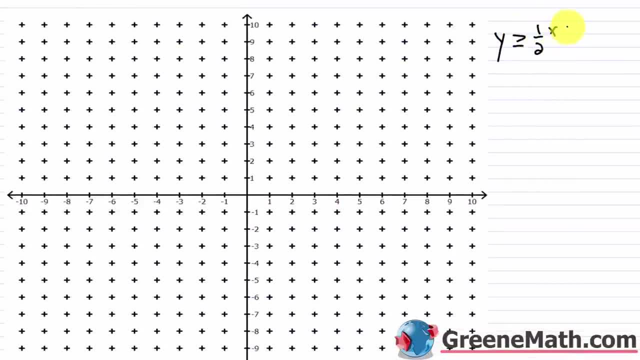 So y is greater than or equal to 1 half x plus 1.. So my boundary line for this- again, remember, all you need to do to make a boundary line is replace this guy with an equal sign. So I would just graph the line: y equals 1 half x plus 1.. 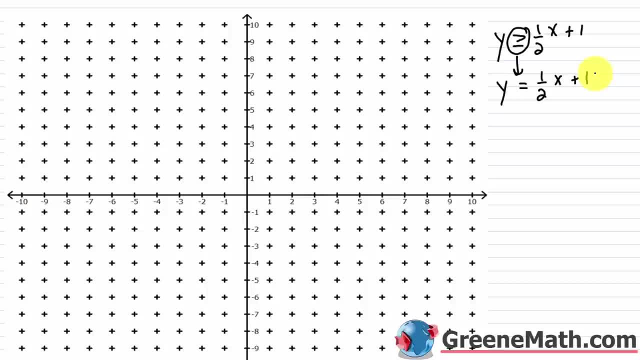 The only thing I need to know is: am I dealing with a strict inequality or a non-strict inequality? Well, this is a greater than or equal to, so it's a non-strict inequality. So we want a solid line. So to graph: y equals 1 half x. 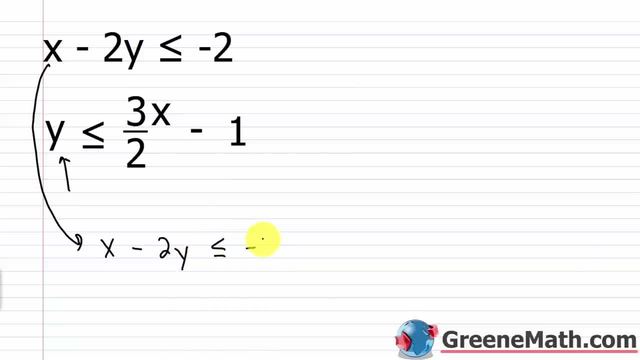 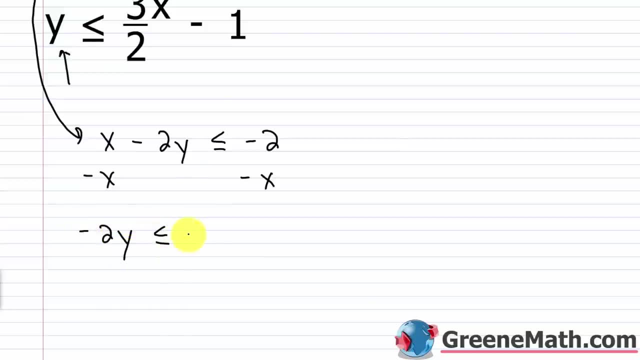 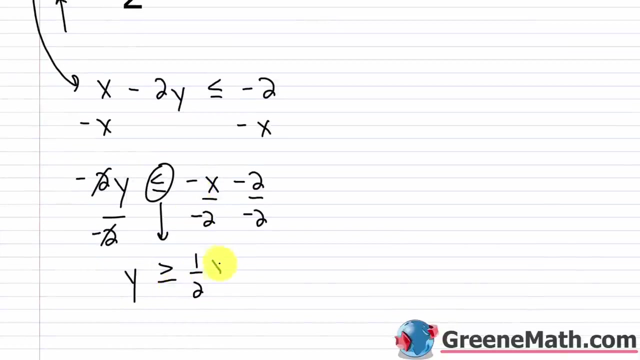 We have x minus 2y is less than or equal to negative 2. So I would subtract x away from each side of the inequality. And I'll have negative 2y. So this is going to be less than or equal to negative x minus 2. Now to get y by itself, I'm going to divide both sides of the inequality by negative 2. So this guy is going to flip. Instead of it being a less than or equal to, it's going to become a greater than or equal to. So this is going to cancel and become y is greater than or equal to negative over negative is positive. So this would be one half x, and then negative 2 over negative 2 would be plus 1. 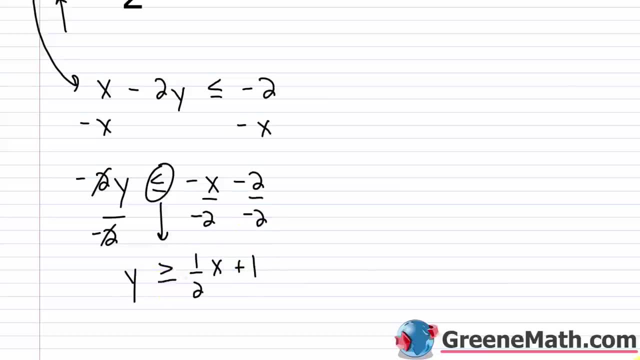 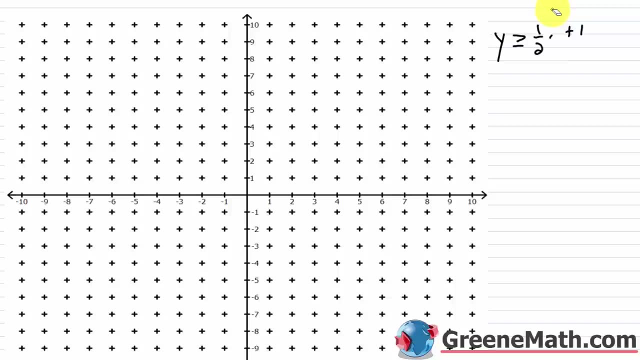 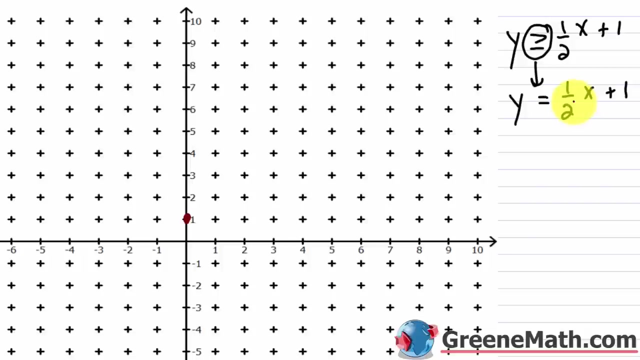 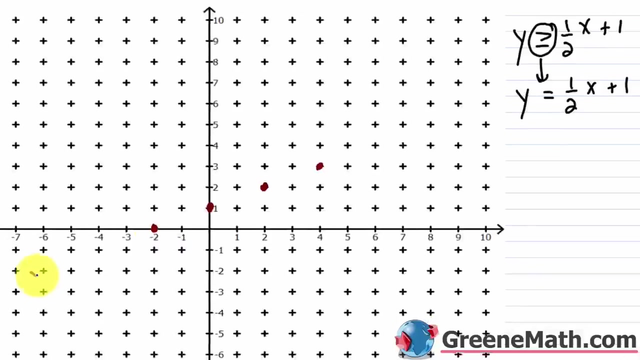 So I've got y is greater than or equal to one half x plus 1. So y is greater than or equal to 1. one-half x plus one. So my boundary line for this, again, remember, all you need to do to make a boundary line is replace this guy with an equal sign. So I would just graph the line y equals one-half x plus one. The only thing I need to know is, am I dealing with a strict inequality or a non-strict inequality? Well, this is a greater than or equal to, so it's a non-strict inequality, so we want a solid line. So to graph y equals one-half x plus one, go to zero comma one, which is right here, and the slope is one-half. So up one, over to the right two, up one, over to the right two, or I can go down one to the left two. Okay, remember, this is going to stay a solid line. 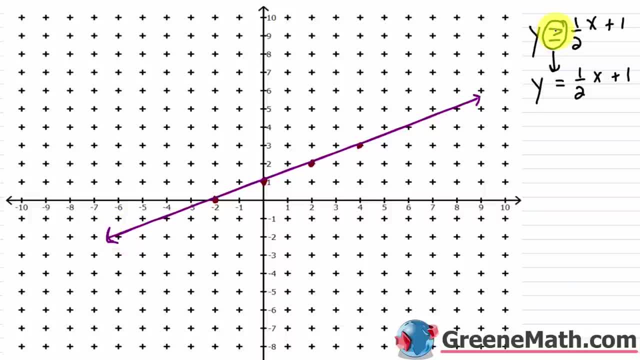 I don't need to break it up at all. And then since y is greater than, right, it's a greater than or equal to, but it's a greater than, 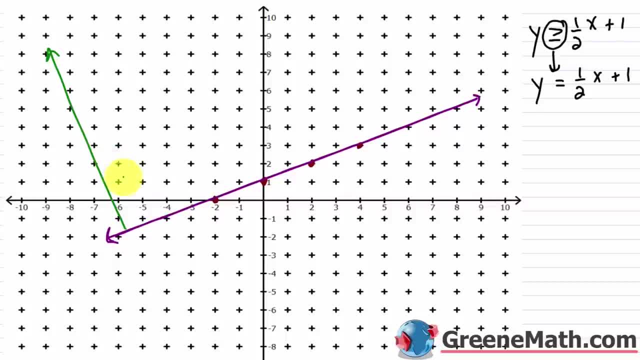 I would shade here above the line. So let me shade above the line. Okay, so that's y is greater than or equal to one-half x plus one. Now we had another one. 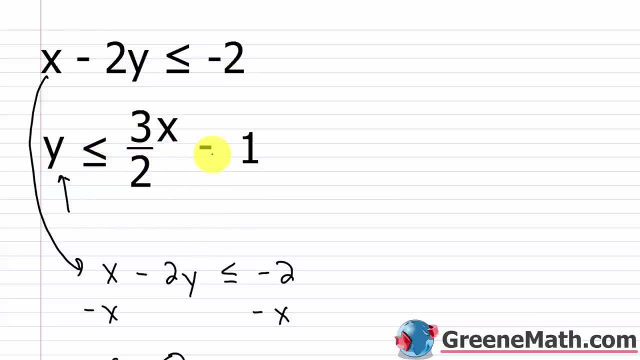 We had y is less than or equal to three-halves x minus one. So y is less than or equal to, again, three-halves x minus one. 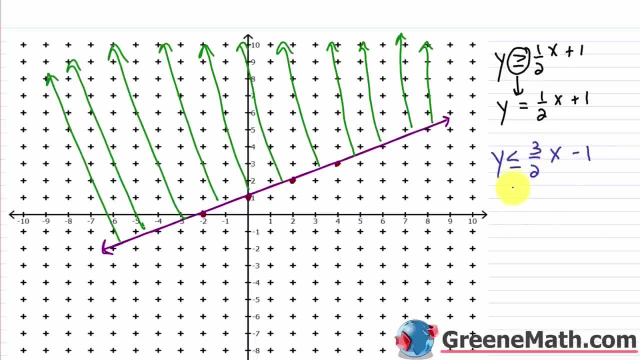 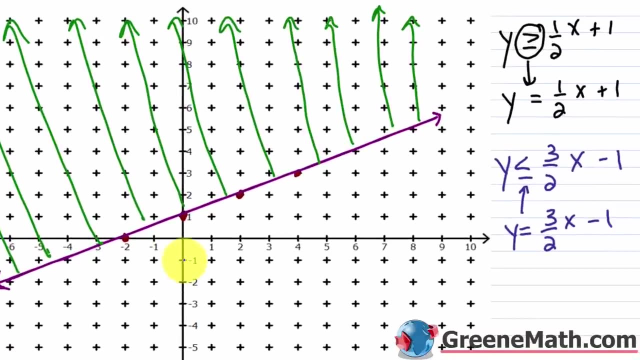 So to graph the boundary line for that, again, I just replace this with equals. So I have y equals three-halves x minus one. And again, this is a non-strict inequality, so we're going to have a solid line. So my y-intercept occurs at zero comma negative one, so it's going to be right here. 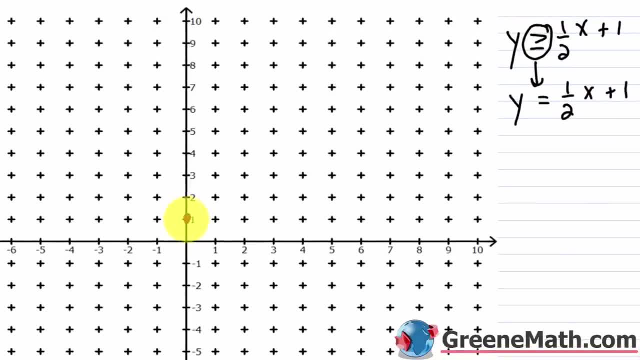 So I'm going to go to 1 half x plus 1,, go to 0 comma 1, which is right here, and the slope is 1 half. so up 1, over to the right 2,, up 1, over to the right 2, or I can go down 1 to the left 2.. 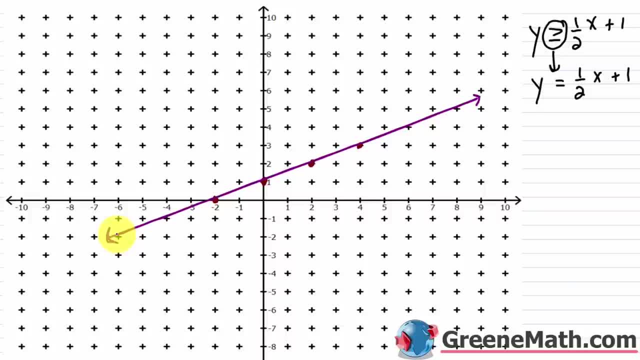 Okay, remember, this is going to stay a solid line, I don't need to break it up at all. And then, since y is greater than right, it's a greater than or equal to, but it's a greater than. I would shade here above the line. 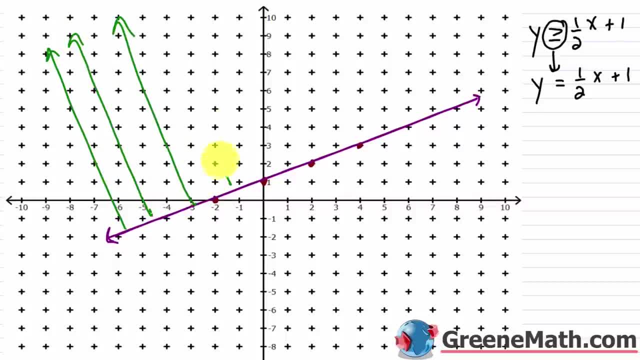 So let me shade above the line. Okay, so that's: y is greater than or equal to, 1 half x plus 1.. Now we had another one. We had: y is less than, or equal to, 3 halves x minus 1.. 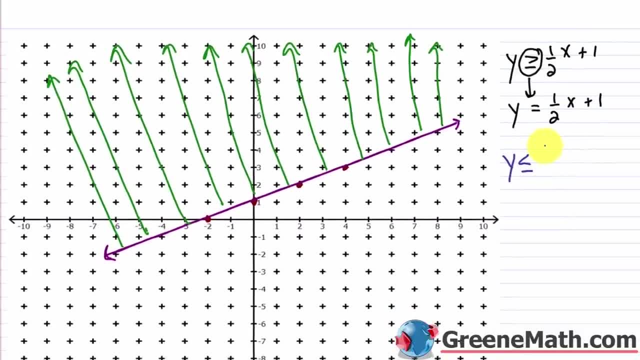 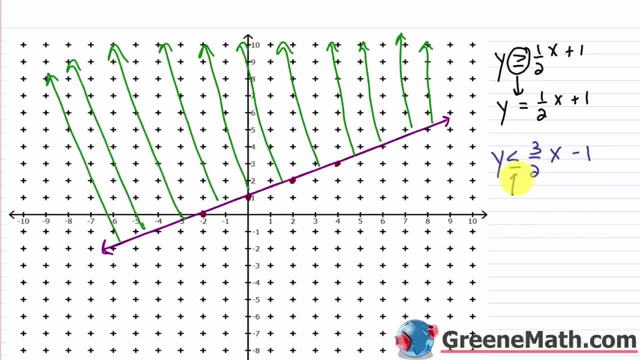 So y is less than or equal to, again, 3 halves x minus 1.. So to graph the boundary line for that, again I just replaced this with: So I have y equals 3 halves x minus 1.. And again, this isn't a non-strict inequality, so we're going to have a solid line. 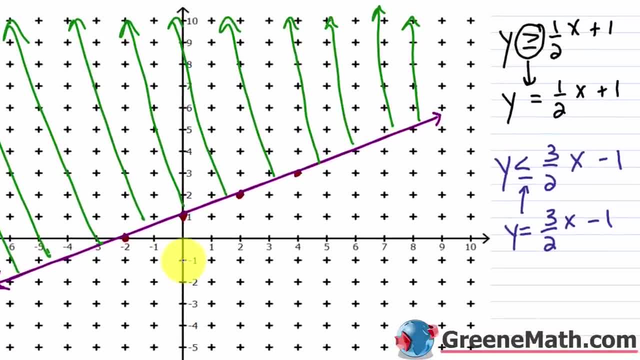 So my y intercept occurs at 0 comma negative 1, so it's going to be right here And my slope is 3 halves. so I'm going to go up 1,, 2,, 3, and then, to the right, 1, 2.. 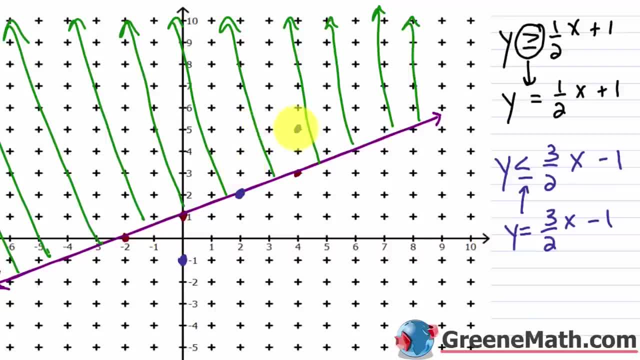 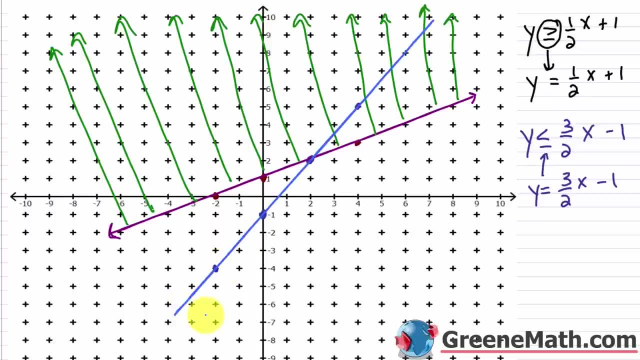 Up 1, 2, 3, to the right, 1, 2.. Or I can go down 1, 2,, 3, to the left, 1, 2.. So this is a less than or equal to, so I'm going to shade below the line. 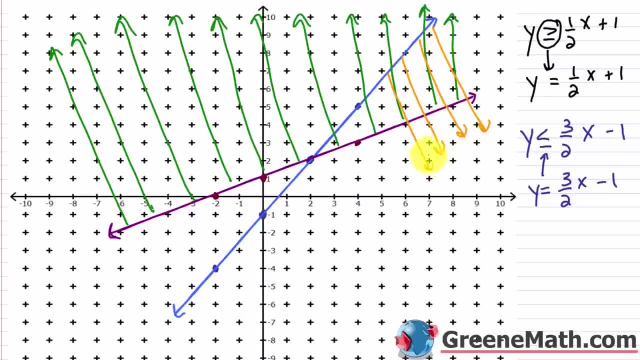 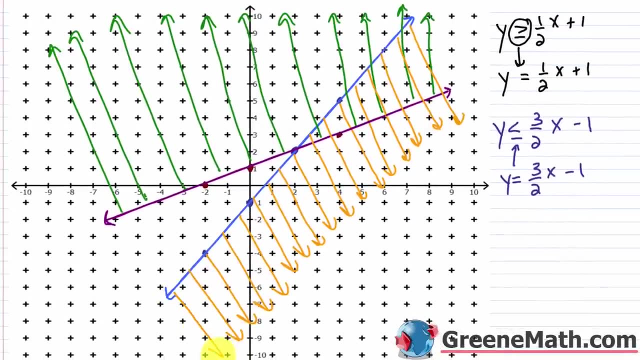 So I'm going to shade below the line here. So where do these two graphs overlap? Well, for this one, compared to our last example, it's kind of a small area. Remember, for this first one, this purple line. it's above right. 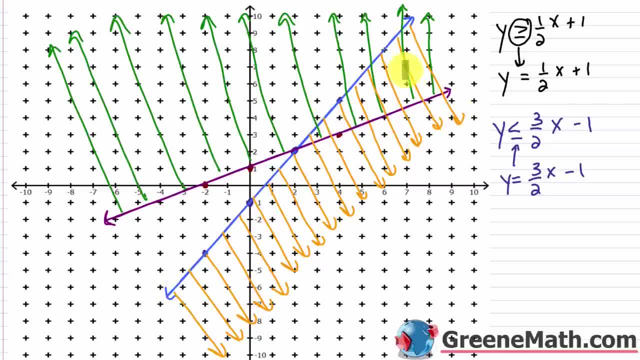 It's above. that's the solution For this blue line. it's below the stuff in orange, it's going down. So the overlap would be this area right here, And I know I'm going over the line a bit, but it would be this: 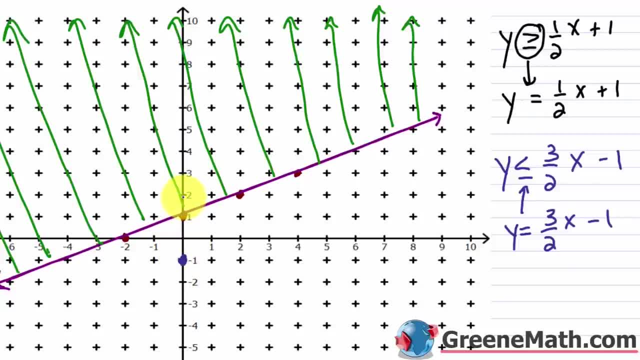 And my slope is three-halves, so I'm going to go up one, two, three, and then to the right one, two. Up one, two, three, to the right one, two. 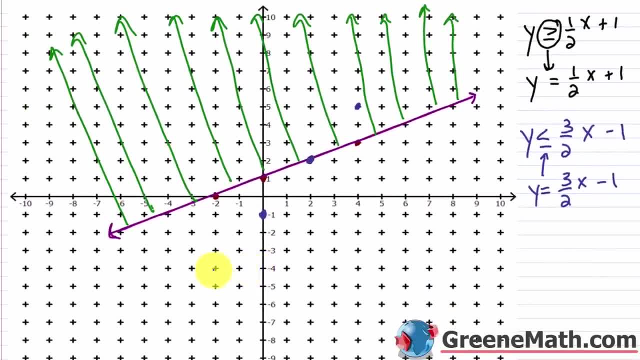 Or I can go down one, two, three, to the left one, two. 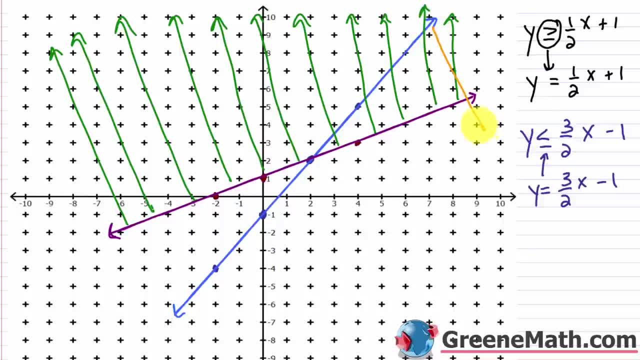 So this is a less than or equal to, so I'm going to shade below the line. So I'm going to shade below the line here. 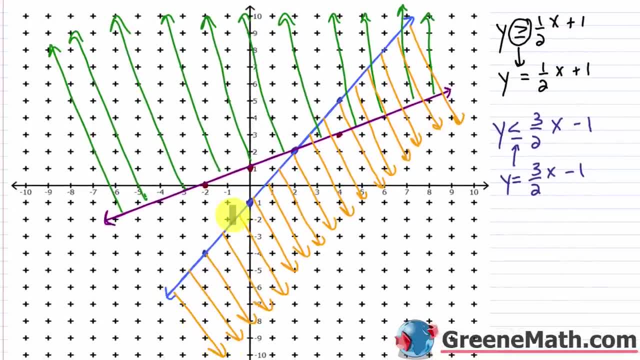 So where do these two graphs overlap? Well, for this one, compared to our last example, it's kind of a small area. Remember, for this first one, this purple line, it's above, right? It's above. That's the solution. For this blue line, it's below. The stuff in orange, it's going down. So the overlap would be this area right here. And I know I'm going over the line a bit, but it would be this. So that's where the overlap is. 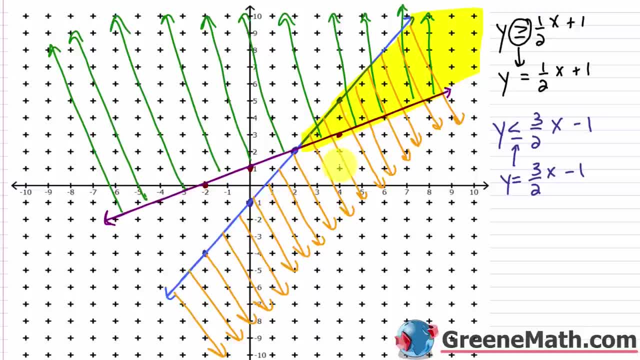 Because anywhere outside of that, you're not going to be in the solution range for the system. 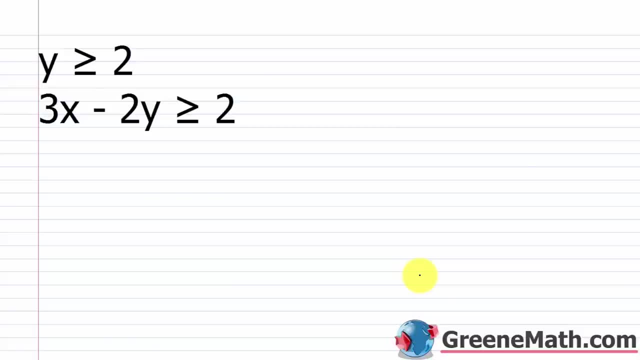 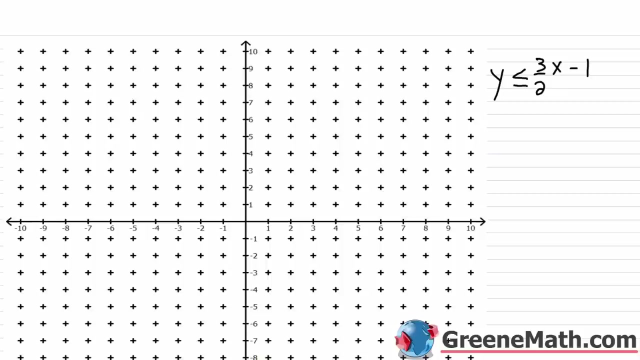 All right, let's take a look at one final problem. We have y is greater than or equal to 2, and then we have 3x minus 2y is greater than or equal to 2. So this one's easy enough to graph. This one right here, I just want to solve it for y. So I'd have negative 2y is greater than or equal to. I would subtract 3x away from both sides of the inequality. So I'd put negative 3x over here, then plus 2. Divide both sides. So I'm going to multiply the inequality by negative 2. And remember, if I do that, I've got to flip the direction of the inequality. So right now, it's a greater than or equal to. We're going to change this to a less than or equal to. So negative 2 over negative 2 is 1. So this would be y. This is less than or equal to negative over negative is positive. So 3 halves x. And then 2 over negative 2 is minus 1. So y is less than or equal to 3 halves x minus 1. Okay, so for the boundary line, I just replace this with equals. 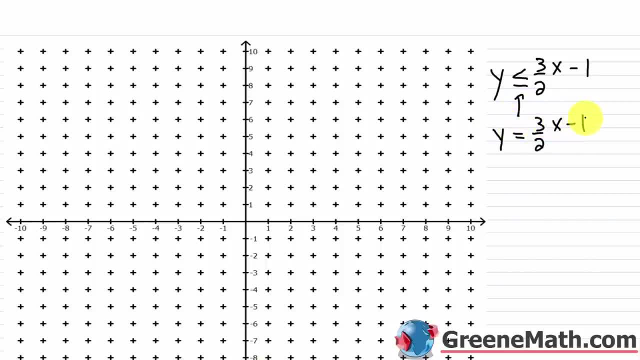 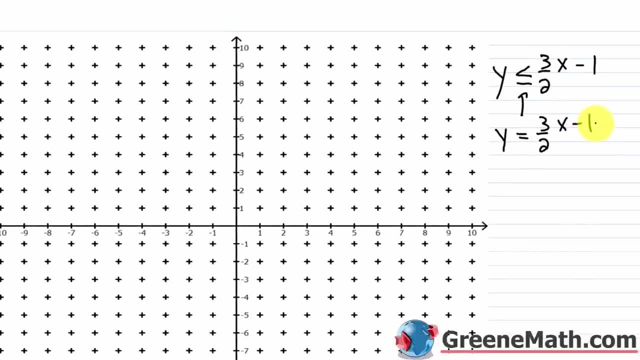 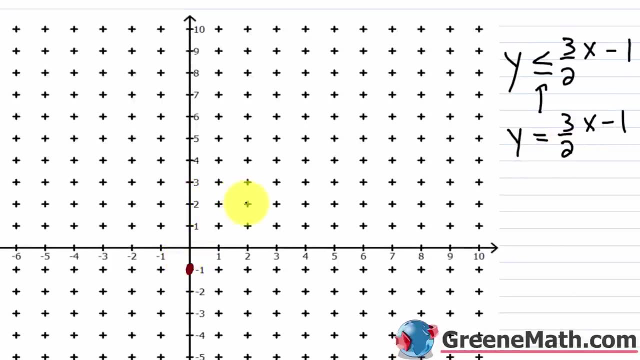 So y equals 3 halves x minus 1. And it's a non-strict inequality. So my boundary line will just be a solid line. So I'm going to go to 0 comma negative 1. So that's right here. That's my y-intercept. And my slope is 3 halves. So up 1, 2, 3 to the right 1, 2. Up 1, 2, 3 to the right 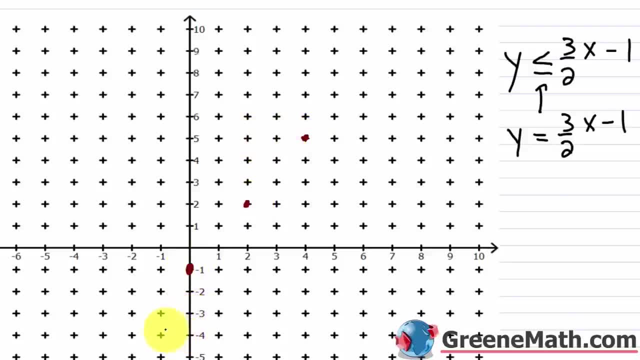 1, 2. Or down 1, 2, 3 to the left 1, 2. 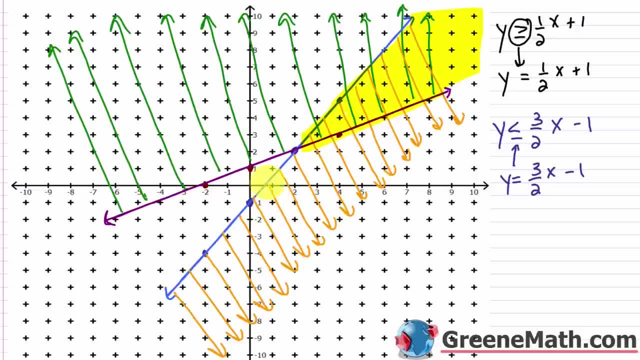 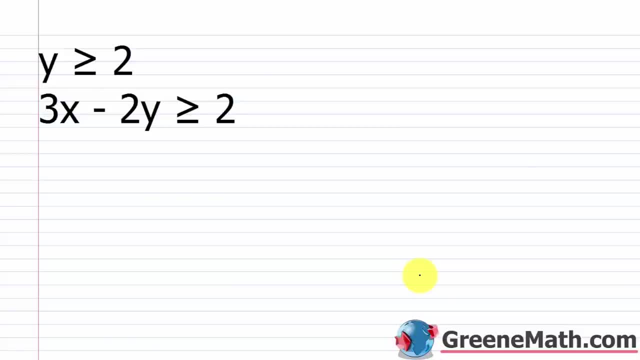 So that's where the overlap is. Anywhere outside of that, you're not going to be in the solution range for the system. All right, let's take a look at One final problem We have. y is greater than or equal to 2.. 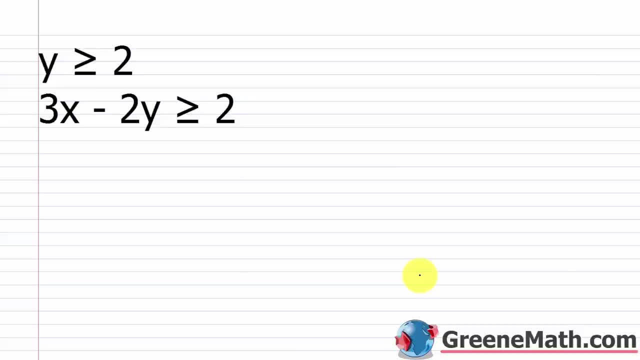 And then we have 3x minus: 2y is greater than or equal to 2.. So this one's easy enough to graph This one right here. I just want to solve it for y. So I'd have negative: 2y is greater than or equal to. 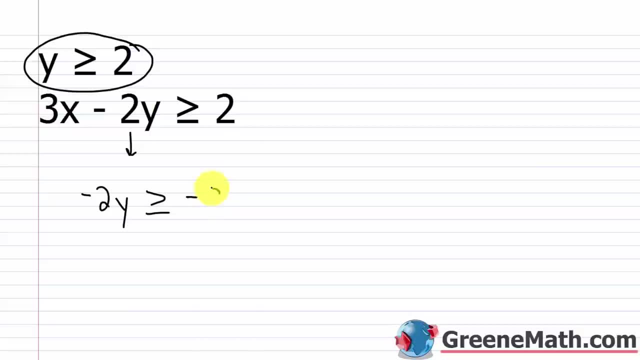 I would subtract 3x away from both sides of the inequality, So I'd put negative 3x over here, then plus 2.. Divide both sides of the inequality by negative 2.. And remember if I do that I've got to flip the direction of the inequality. 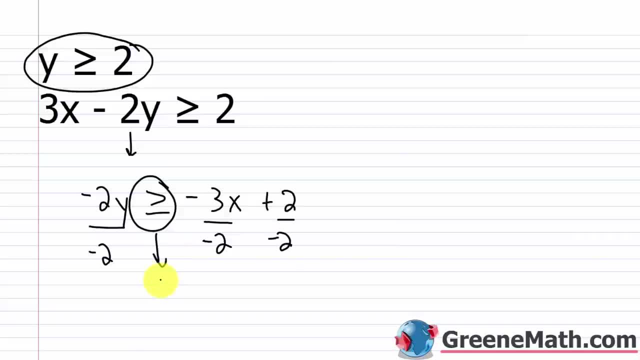 So Right now it's a greater than or equal to. We're going to change this to a less than or equal to, So negative 2 over negative 2 is 1.. So this would be y. This is less than or equal to negative over negative is positive. 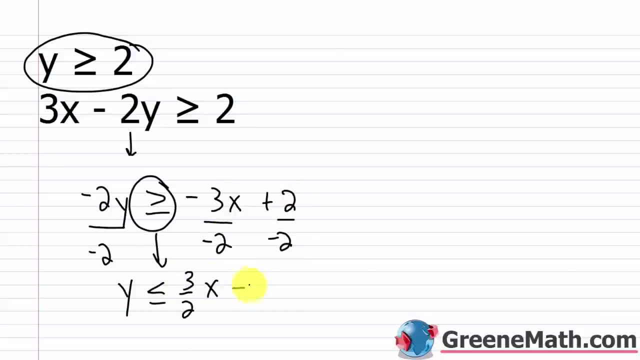 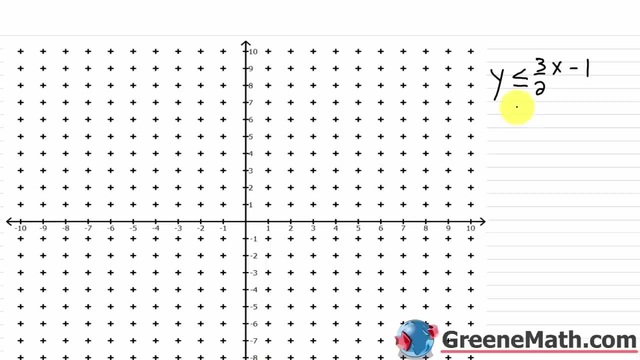 So 3 halves x And then 2 over negative, 2 is minus 1.. So y is less than or equal to, 3 halves x minus 1.. OK, so for the boundary line, I just replace this with equals. So y equals 3 halves x minus 1.. 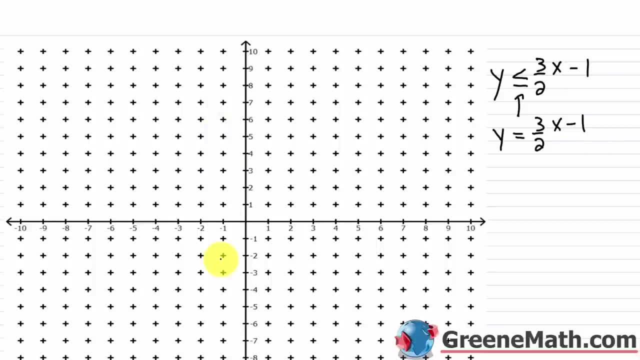 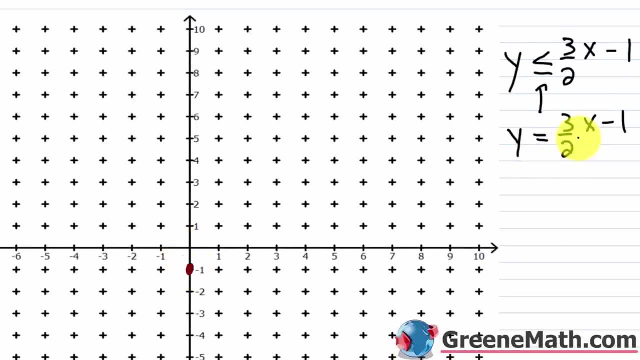 And it's a non-strict inequality. So my boundary line will just be a solid line. So I'm going to go to 0 comma negative 1.. So that's right here. That's my y intercept And my slope is 3 halves. 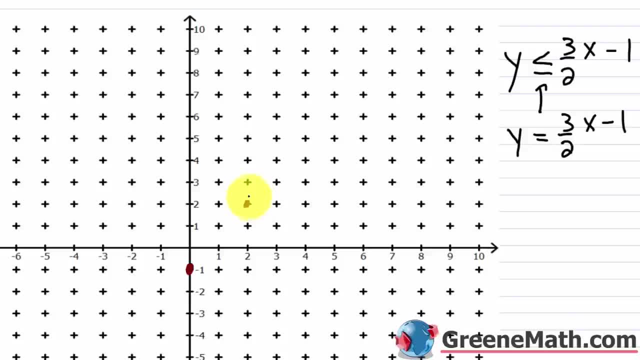 So up, 1, 2, 3, to the right, 1, 2.. Up, 1, 2, 3, to the right, 1, 2.. Or down, 1, 2, 3, to the left, 1, 2.. 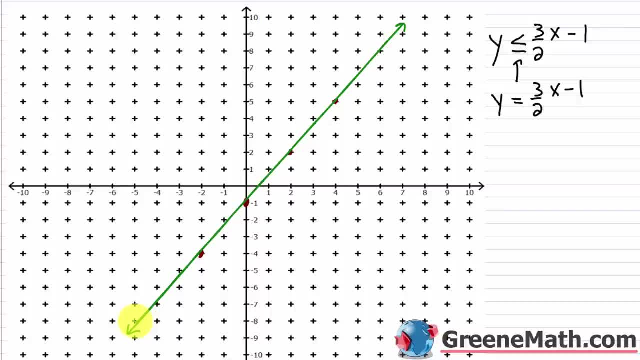 Again, this is a solid line, So no need to take the eraser out. And it's y is less than or equal to. So with a less than or less than or equal to, I shade below the line. So I would shade everything going this way. 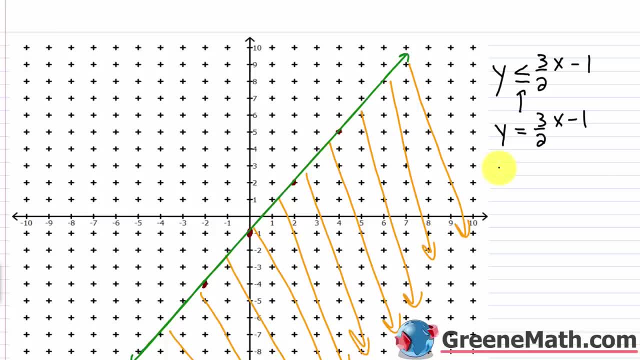 Now the other one we had was y is greater than or equal to 2.. So y is greater than or equal to 2.. So the boundary line there is at y equals 2.. And again, non-strict inequality, So it's a solid line. 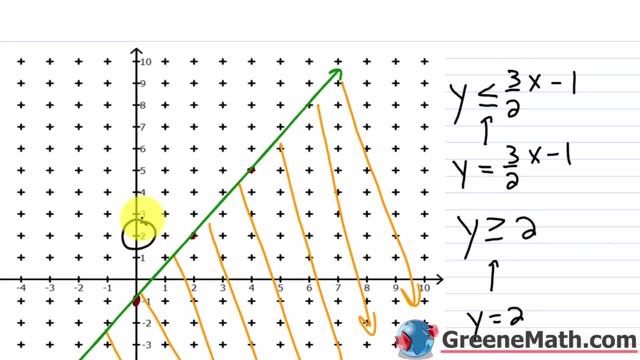 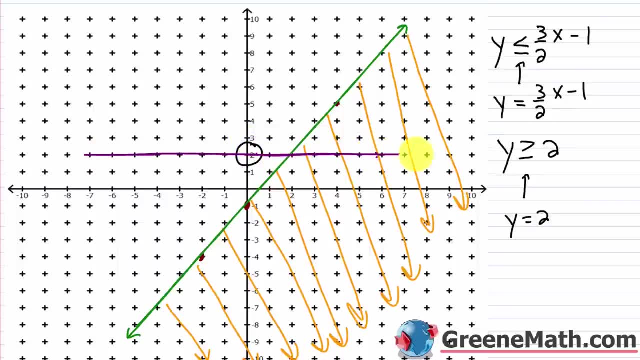 So to graph y equals 2.. I just find 2 on the y-axis And I draw a horizontal line. Okay, And then this is a greater than or equal to. So I shade above the line. So I'm going to shade everything going above the line. 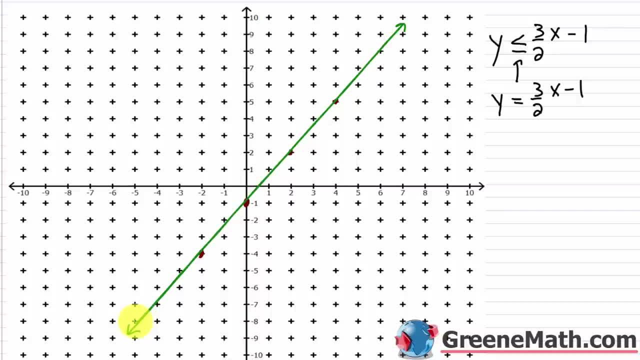 Again, this is a solid line. So I'm going to go to 0 comma negative 1. So that's right here. That's a solid line. So no need to take the eraser out. And it's y is less than or equal to. So with a less than or less than or equal to, I shade below the line. So I would shade everything going this 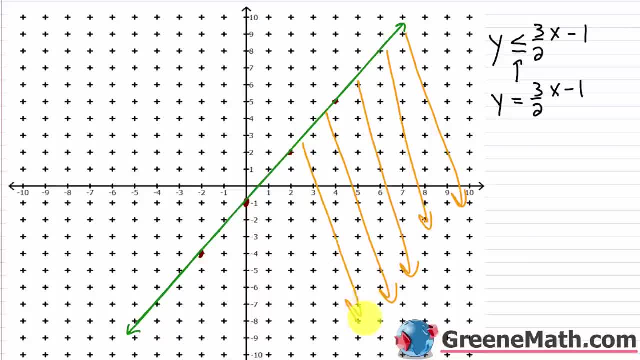 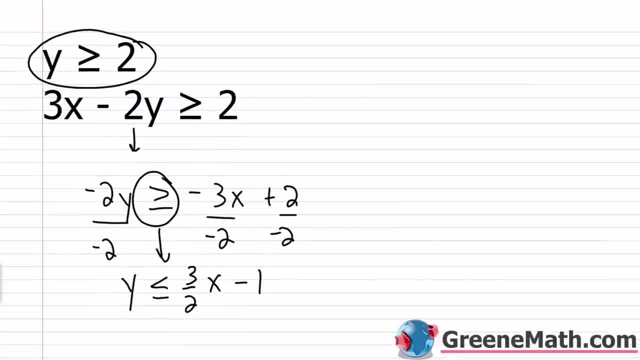 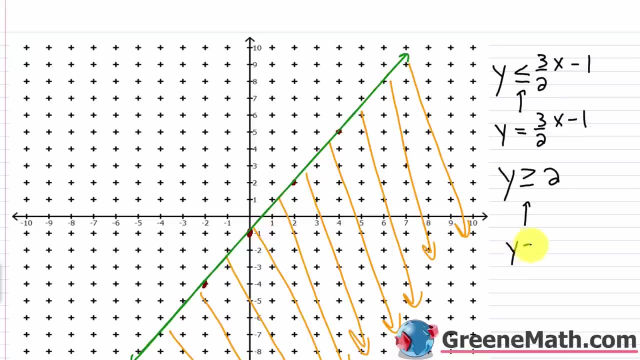 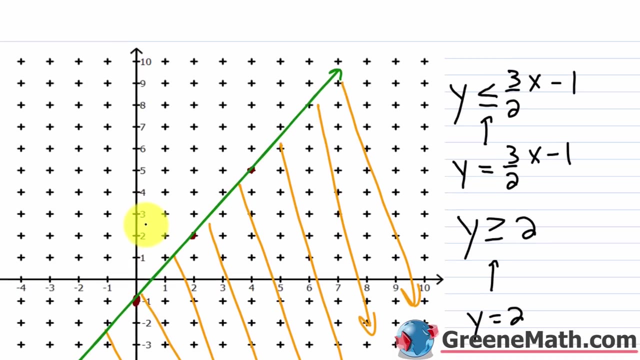 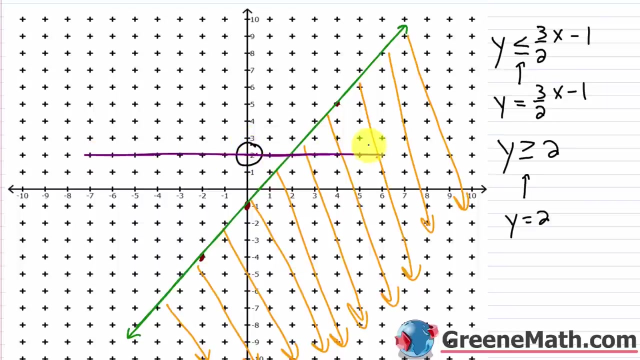 way. Now the other one we had was y is greater than or equal to 2. So y is greater than or equal to 2. So the boundary line there is at y equals 2. So I'm going to go to 0 comma negative 1. So again, non-strict inequality. So it's a solid line. So to graph y equals 2, I just find 2 on the y-axis. And I draw a horizontal line. And then this is a greater than or equal to. So I 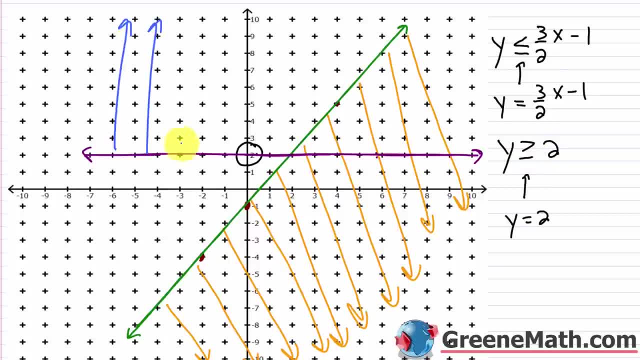 shade above the line. So I'm going to shade everything going above the line. 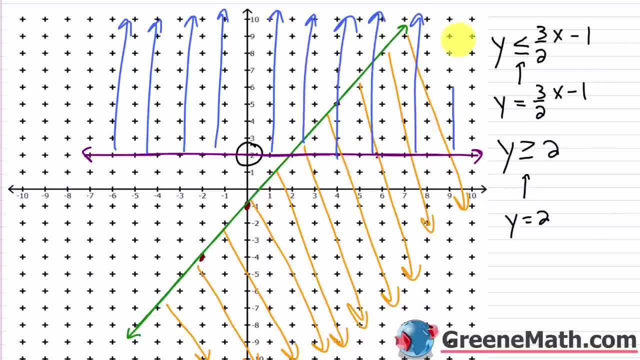 And so where's my area of intersection? Where do the graphs overlap? Well, it's this area going like this. Everywhere I'm highlighting here would be the area that's a solution for both. So in real life, this is an infinite area. But just to get a picture of it, we can see what we have here. And I went a little bit over the line here. It's just got to be exactly on that green line and on that purple line. And so I'm going to go to 0 comma negative 1. So I shade above the line. Those would be part of the solution for the system, but nothing above that, okay? So there's your solution for the system, that area that is highlighted. 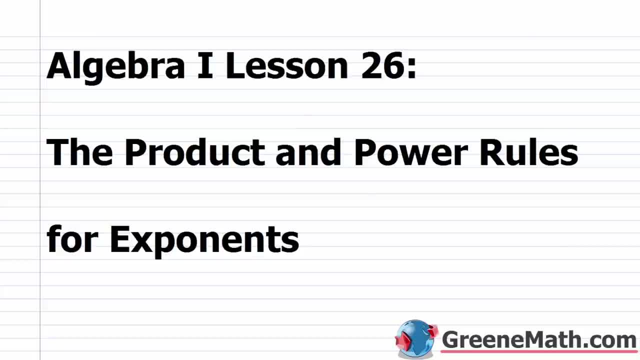 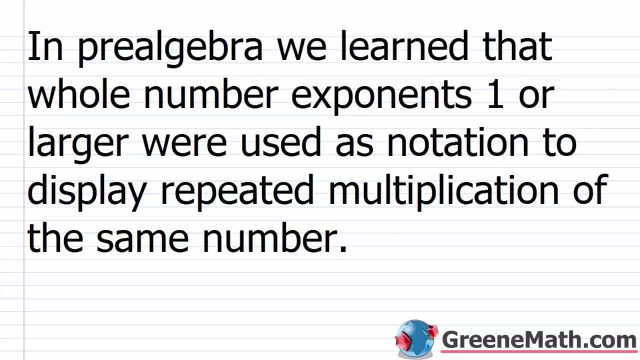 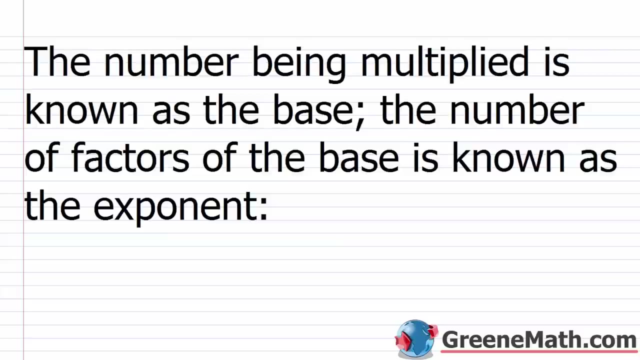 Hello, and welcome to Algebra 1, Lesson 26. In this video, we're going to learn about the product and power rules for exponents. So back in pre-algebra, we learned that whole number exponents, one or larger, were used as notation to display repeated multiplication of the same, number. I want you to recall that the number being multiplied is known as the base, whereas the number of factors of the base is known as the exponent. So for example, 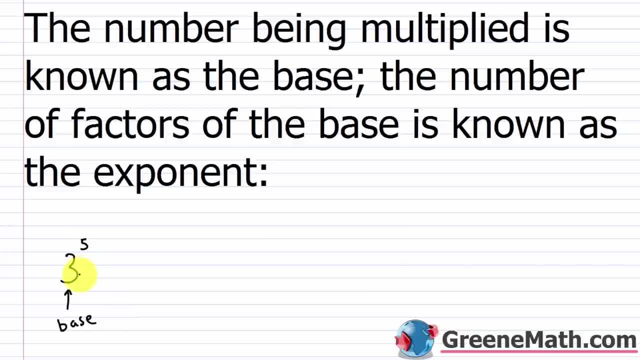 This, again, is the number that's going to be multiplied by itself. Then this little guy up here, this 5, is going to be multiplied by itself. So this little guy up here, this 5, 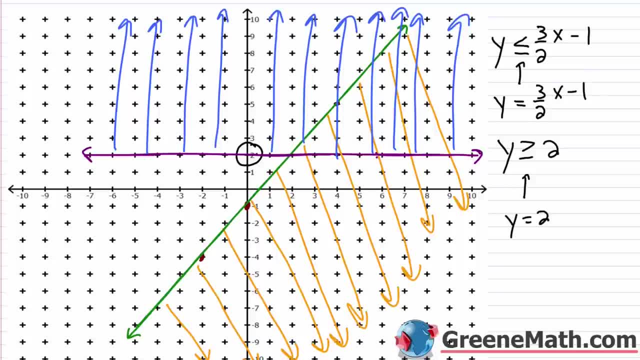 And so where's my a Area of intersection? Where do the graphs overlap? Well, it's this area, going like this Everywhere. I'm highlighting here would be the area that's a solution for both. So, in real life, this is an infinite area. 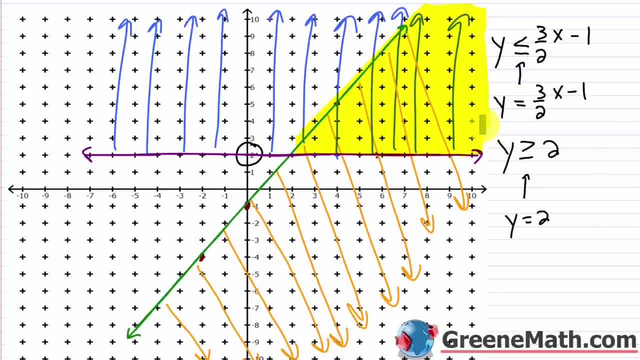 But just to get a picture of it, we can see what we have here, And I went a little bit over the line here. It's just got to be exactly on that green line and on that purple line. Those would be part of the solution for the system, but nothing above that. 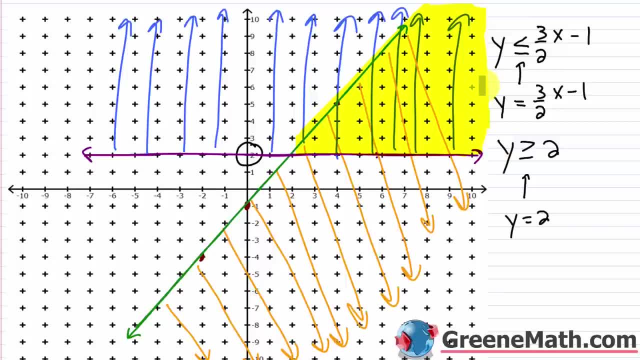 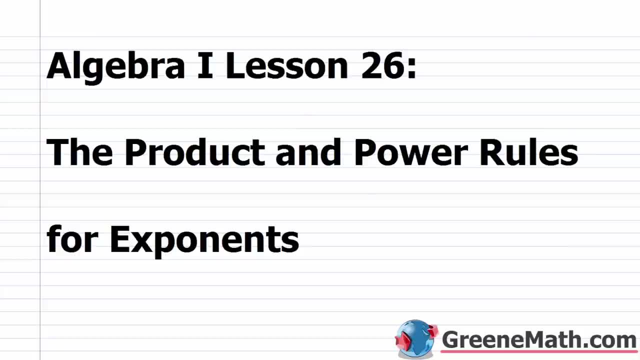 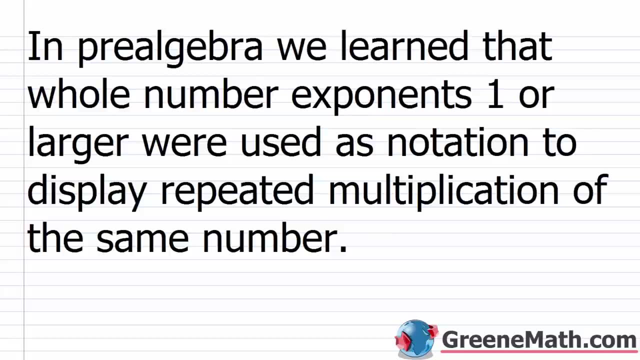 Okay, so there's your solution for the system, that area that is highlighted. Hello and welcome to Algebra 1, Lesson 26.. In this video we're going to learn about the product and power rules for exponents. So back in pre-algebra we learned that whole number exponents: one or larger. 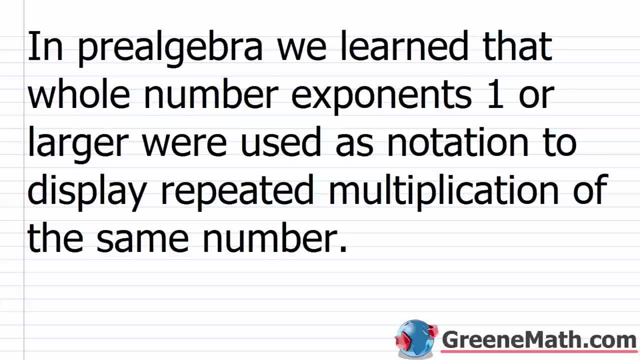 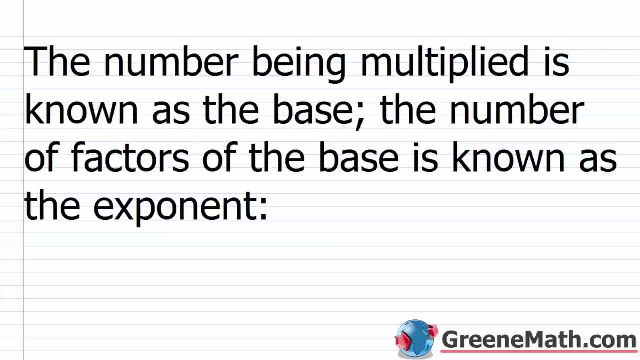 were used as notation to display repeated multiplication of the same number. I want you to recall that the number being multiplied is known as the base, Whereas the number of factors of the base is known as the exponent. So, for example, let's say we had something like 3 to the 5th power. 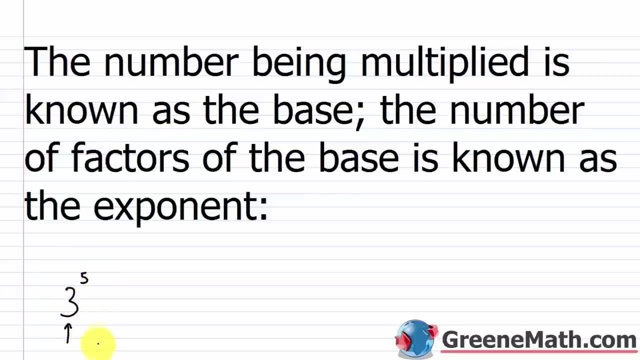 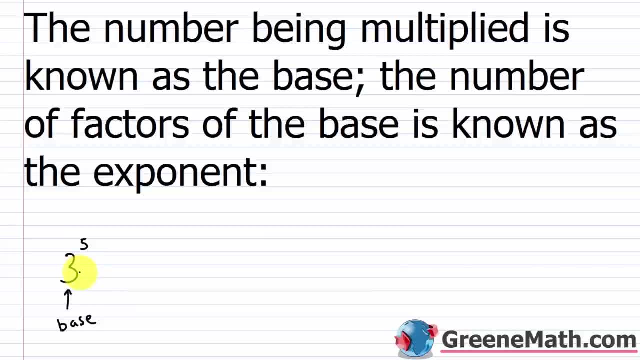 3,. the bigger number is known as the base. This again is the number that's going to be multiplied by itself. Then this little guy up here, this 5, is known as the exponent. This again tells us how many factors of the base that we have. 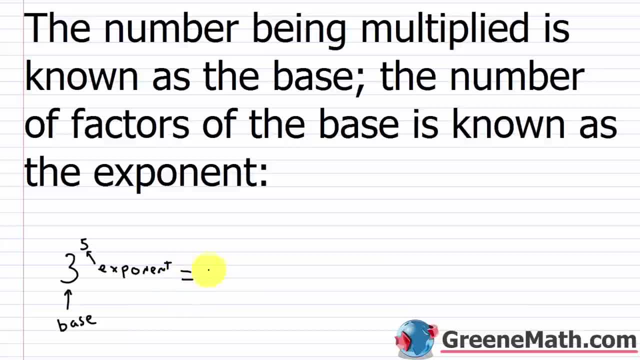 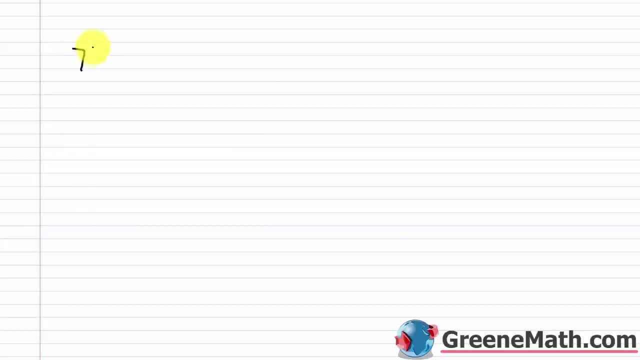 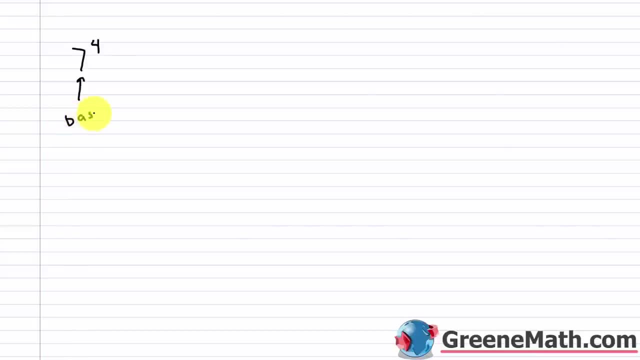 Again 7, the bigger number is the base And then 4, the little number up here is the exponent, And again this is telling me. I have 4 factors of 7.. So this is 7 times 7 times 7 times 7.. 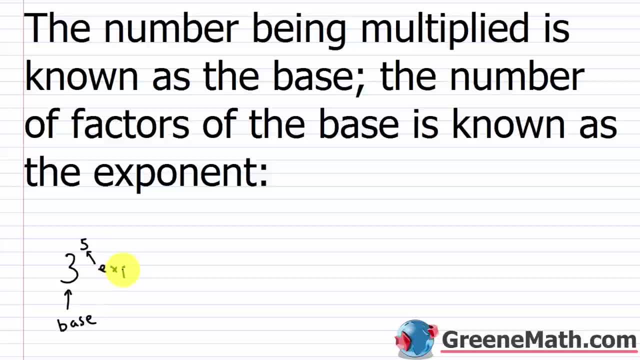 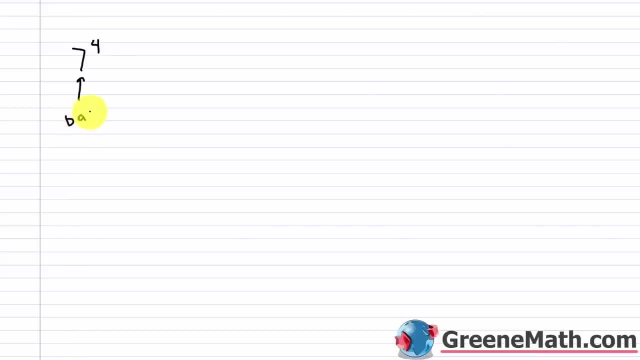 Again, 7, the bigger number, is the base. And then 4, the little number up here, is the exponent. 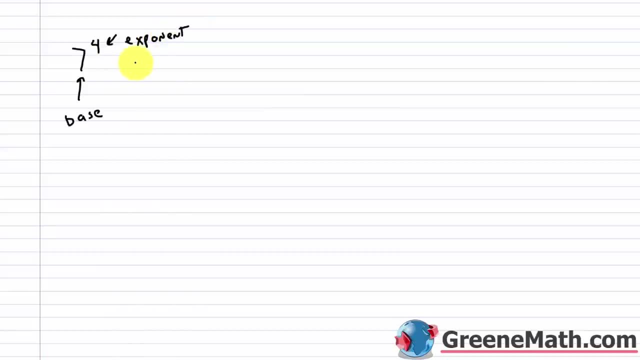 And again, this is telling me I have 4 factors of 7. So this is 7 times 7 times 7 times 7. 1, 2, 3, 4 factors of 7. Now we can also do this with variables. And in pre-algebra, we didn't talk 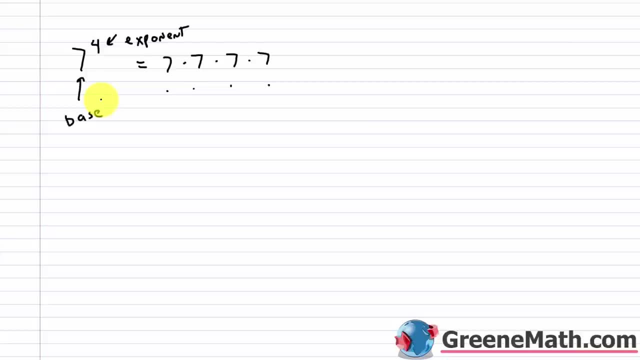 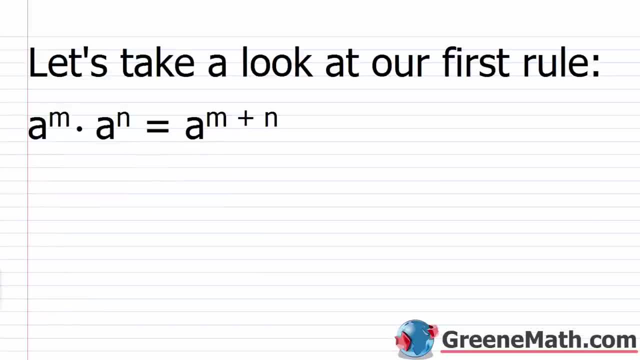 5 6 factors of X so in a short time we're gonna start working with polynomials and before we get to this topic we have to have a complete 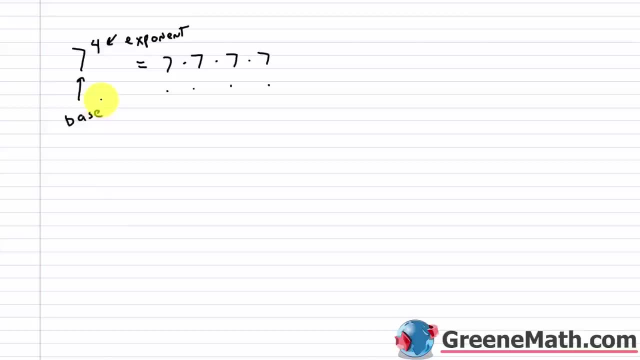 1,, 2,, 3,, 4 factors of 7.. Now we can also do this with variables, And in pre-algebra we didn't talk about variables at all. But it would be the same thing if I said: OK, I have x to the 6th power. 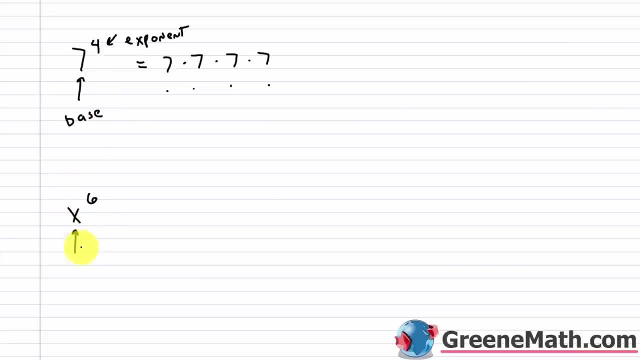 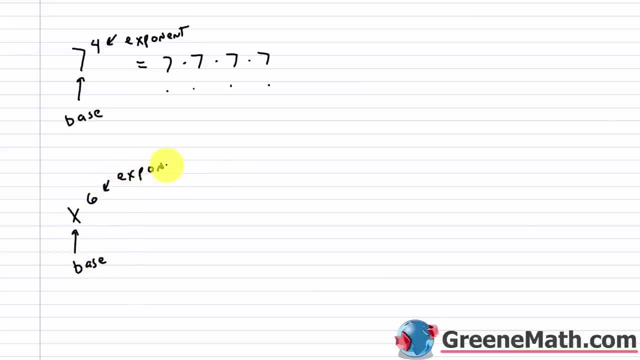 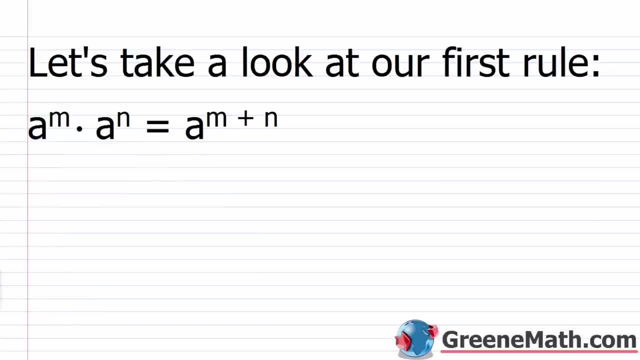 So in a short time we're going to start working with polynomials, And before we get to this topic, we have to have a complete understanding of how to work with exponents. It is very, very critical to your success with polynomials. 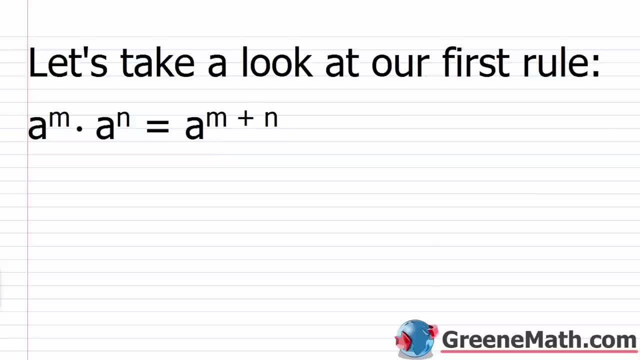 So the first thing I'm going to teach you is called the product rule for exponents. So it's very, very simple And it's very, very intuitive. We have a to the power of m times a to the power of n is equal to a to the power of m plus n. 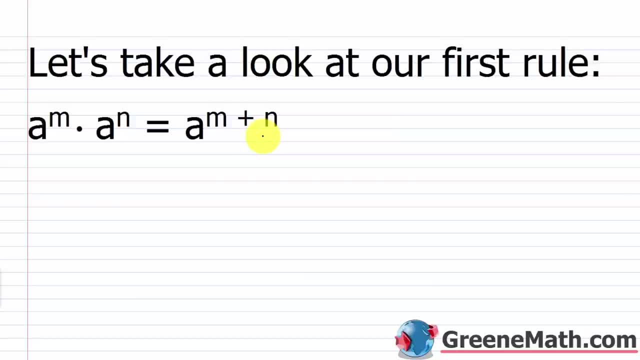 And I know some of you will have a glazed over look when your eyes are closed right now- But essentially something you'd see in your textbook, to kind of translate into something you can understand when we multiply two numbers or expressions in exponent form with the same base: 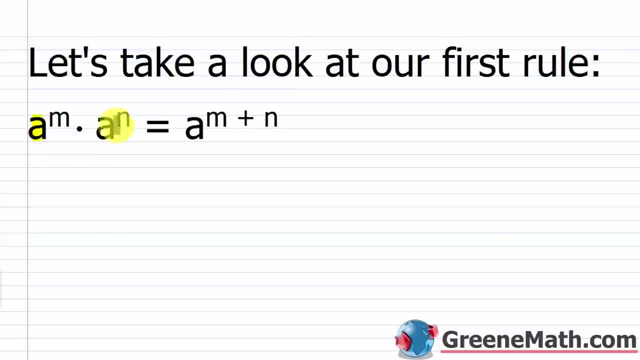 So that's the key here: with the same base. Here I have a And then I have the same a here. So what we do is we keep the base the same, So I don't change a at all, And then I just add the exponents. 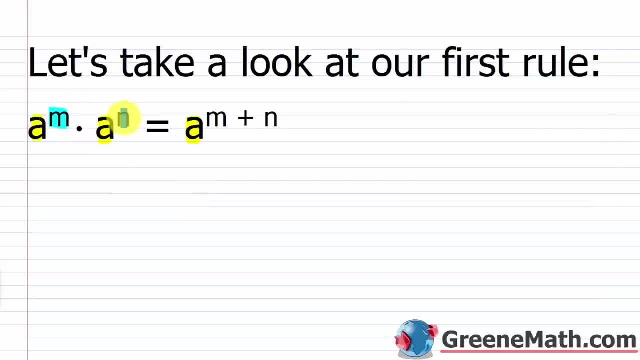 So you notice how the exponent here is m and the exponent here is n And we have m plus n right there. So even if that doesn't make sense right away, let's take a look at some examples and kind of let it set in a little bit. 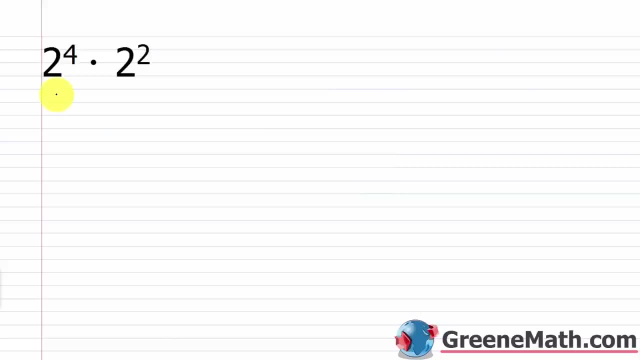 So we have 2 to the fourth power times 2 squared. So again we're looking for the same base. So I have a base of 2. And I have a base of 2. So it's the same base. It's got to be the same number. 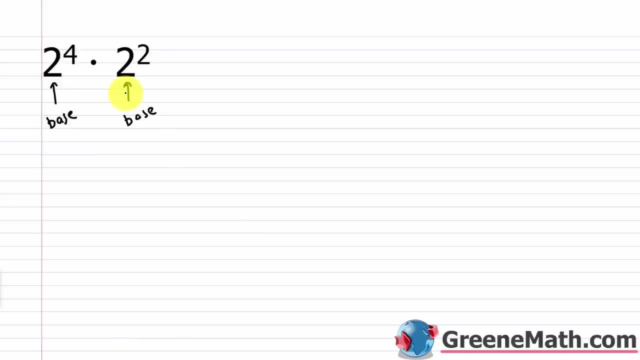 If 1 is 2 and 1 is, let's say, 8, that's not going to work. The base has to be the same. So what I'm going to do is I'm going to keep that base the same. 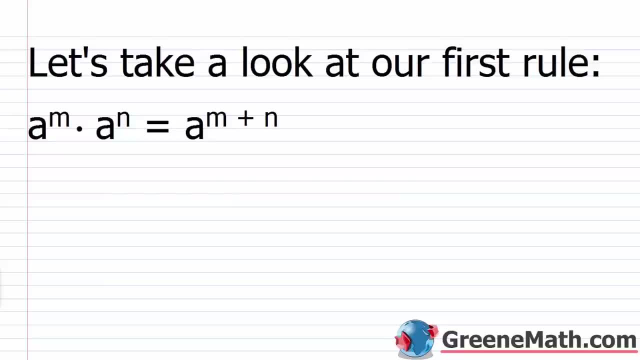 understanding of how to work with exponents it is very very critical to your success with polynomials so the first thing I'm gonna teach you is called the product rule for exponents so it's very very simple and it's very very intuitive we have a to the power of M times a to the power of P and it's very very intuitive we have a to the power of M of n is equal to a to the power of m plus n and i know some of you will have a glazed over look on your eyes right now but essentially something you'd see in your textbook to kind of translate into something you can understand when we multiply two numbers or expressions in exponent form with the same base so that's the key here with the same base here i have a and then i have the same a here so what we do is we keep the base the same so i don't change a at all and then i just add the exponents so you notice how the exponent here is m and the exponent here is n and we have m plus n right there so even if that doesn't make sense right away let's take a look at some examples and kind of let it set in a little bit so we have two to the fourth power times two squared so again we're looking for the same base so i have a base of two so 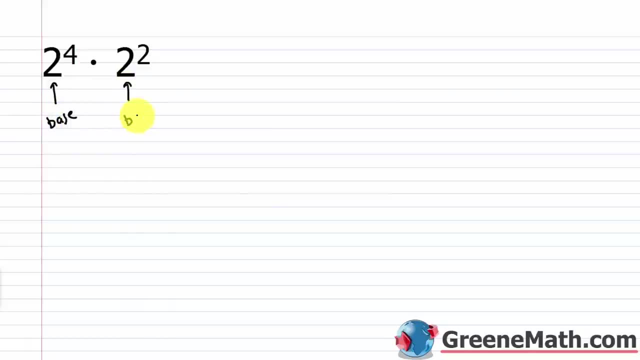 so I have a base of two so it's the same base it's got to be the same number if one is two and one is let's say eight that's not going to work the base has to be the same so what i'm going to do is i'm going to keep that base the same so i'm not going to change it so it's going to stay as a two and then i'm just going to add the exponents so i have an exponent here four and i have an exponent 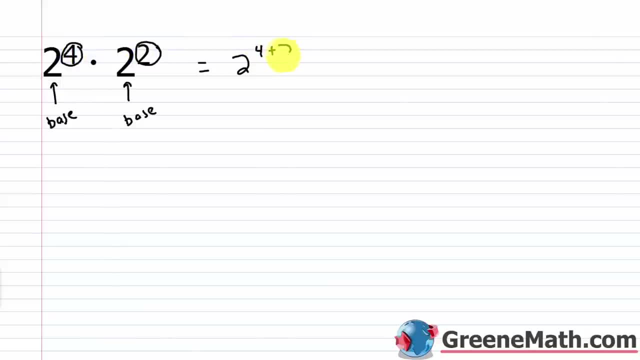 here of two so i would do four plus two which is six so this is two to the sixth power now where does this come from 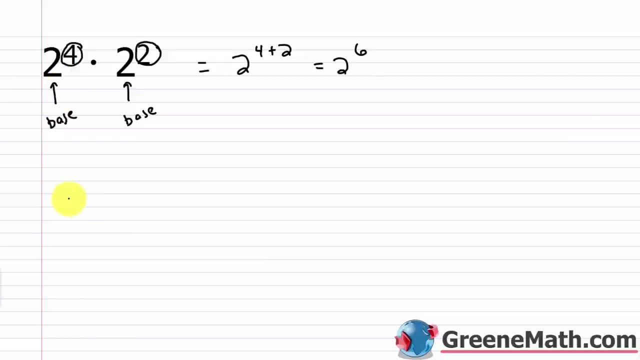 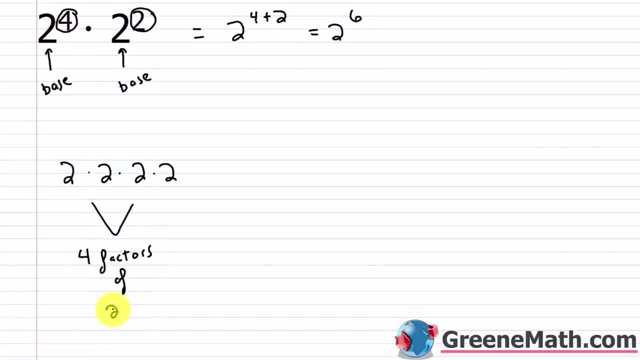 let's think about this for a second if I have two to the fourth power thats two times two times two times two it's four factors of two now if i multiply that by two squared i am essentially just multiplying it by another two factors so two times two so this is two factors two factors of two so to figure out that our equation would be out how many total factors I have I just add the number of factors I have here which was four 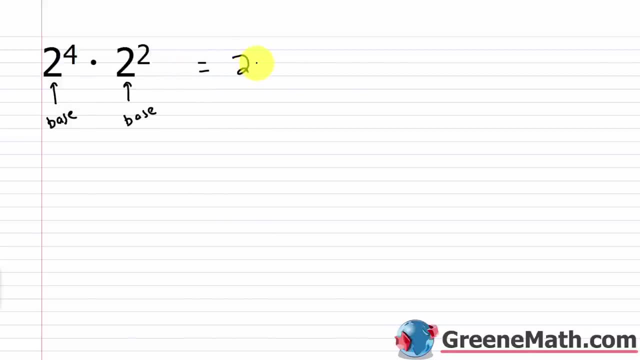 So I'm not going to change it, So it's going to stay as a 2.. And then I'm just going to add the exponents. So I have an exponent here of 4. And I have an exponent here of 2.. 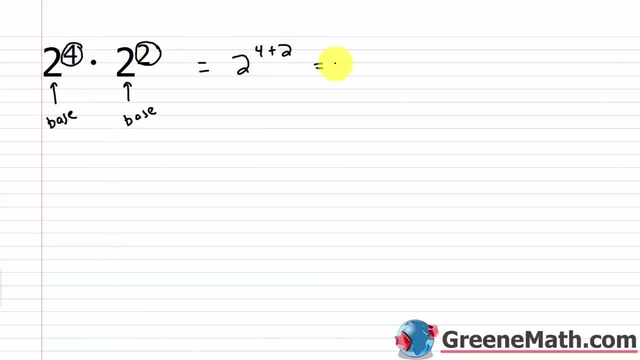 So I would do 4 plus 2, which is 6.. So this is 2 to the sixth power. Now, where does this come from? Let's think about this for a second. If I have 2 to the fourth power, that's 2 times 2 times 2 times. 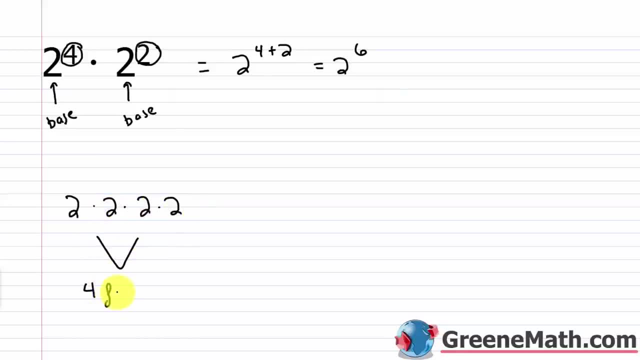 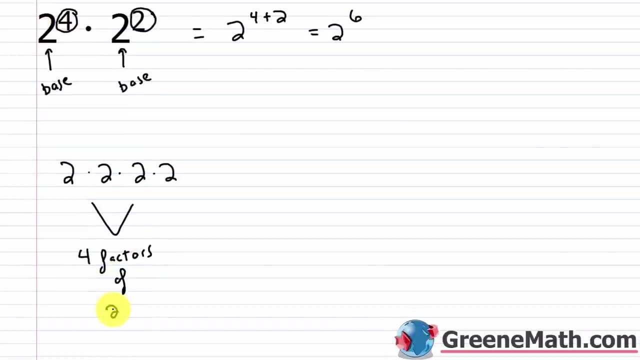 2.. It's four factors, So I have 2 to the sixth power of 2.. Now if I multiply that by 2 squared, I'm essentially just multiplying it by another two factors. So 2 times 2.. So this is two factors. 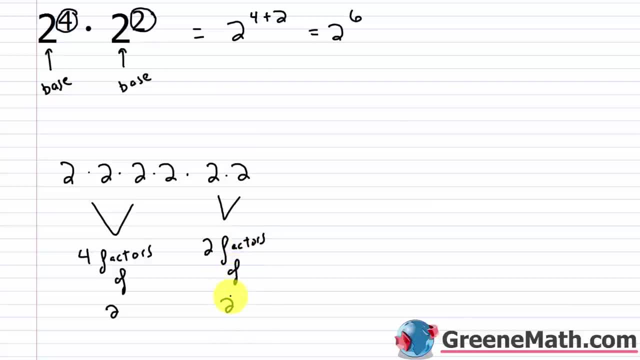 Two factors of 2.. So to figure out how many total factors I have, I just add the number of factors I have here, which was 4, given to me by this exponent, to the number of factors I have here, which is 2, given to me. 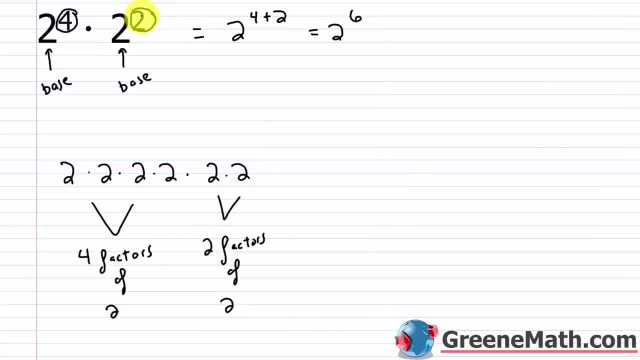 by this exponent. So doesn't it make more sense just to go through and just keep the base the same, the number that's being multiplied by itself, and just add the exponents Right, Because that's going to tell me how many total factors? 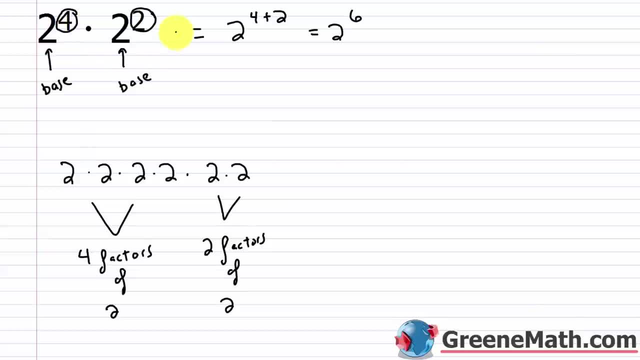 of this base that I'm going to have in the end. This is a lot easier to do than writing all this out every time and saying, OK, this is 2 to the sixth power And you can go through and evaluate this if you want. 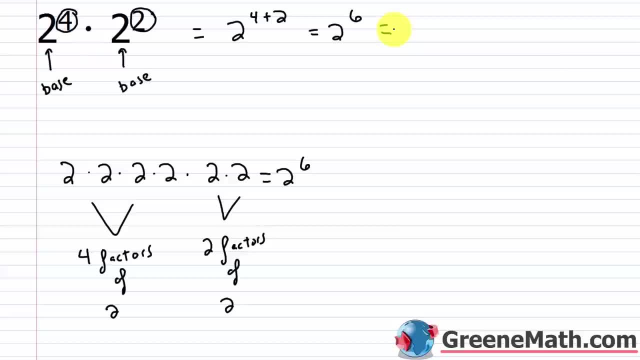 You don't have to. Usually at this stage of the game, they just want you to write 2 to the sixth power, But 2 to the sixth power. 6th power is 2 times 2, which is 4, times another 2,, which is 8, times 2 again, which is 16,. 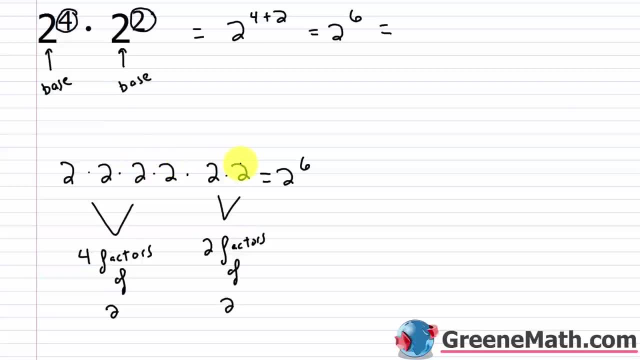 times 2 once more, which is 32,. and times 2 one more time, which is 64.. And, by the way, by the time you get out of Algebra 1, you're going to know up to 2, to the 8th power. 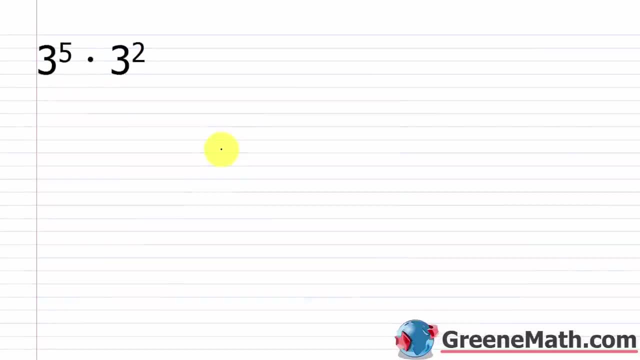 by heart because you're going to use it so often. All right, let's take a look at another one. We have 3 to the 5th power times 3 squared. So again, I'm looking to see that I have the same base. So 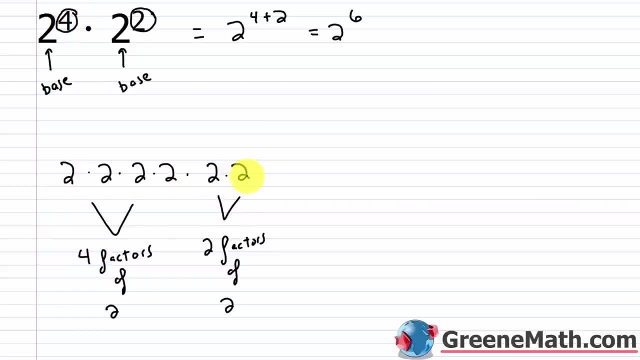 given to me by this exponent to the number of factors I have here which is two given to me by 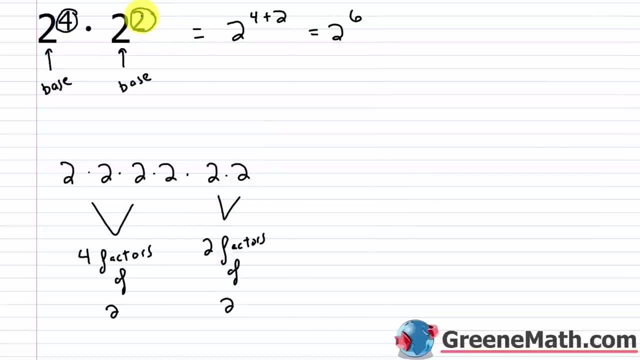 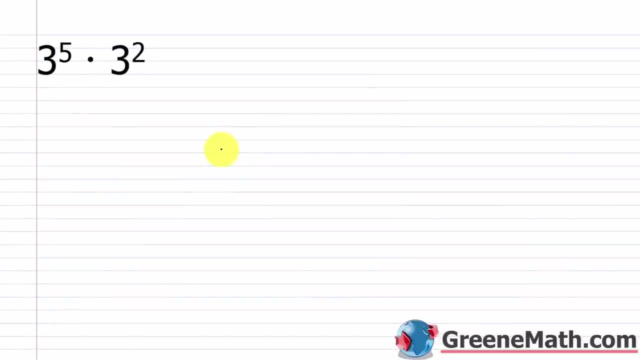 this exponent. So doesn't it make more sense just to go through and just keep the base the same the number that's being multiplied by itself and just add the exponents right because that's going to tell me how many total factors of this base that I'm going to have in the end. This is a lot easier to do than writing all this out every time and saying okay this is two to the sixth power and you can go through and evaluate this if you want you don't have to usually at this stage of the game they just want you to write two to the sixth power but two to the sixth power is two times two which is four times another two which is eight times two again which is 16 times two once more which is 32 and times two one more time which is 64. And by the way by the time you get out of algebra one you're going to know you're going to know up to two to the eighth power by heart because you're going to use it so often. All right let's take a look at another one. We have three to the fifth power times three squared. So again I'm looking to see that I have the same base so this is the same as this so there's my base and there's my base. Here's my exponent and here's my other exponent. Now the rule tells me if I have the same base which I do here I'm going to keep the base the same so just write a three and then I'm 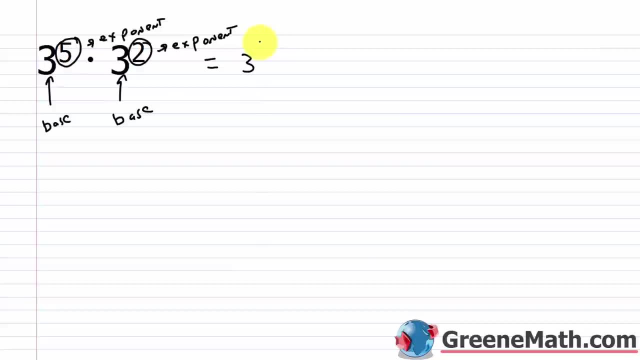 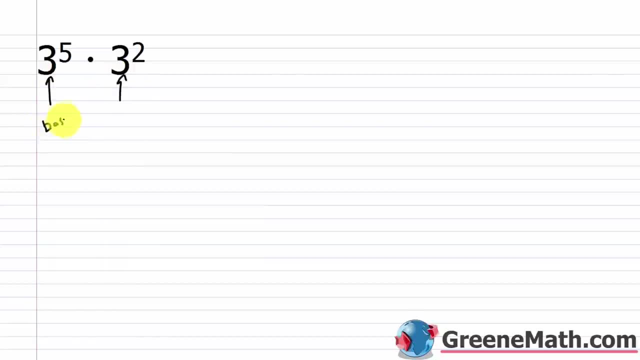 this is the same as this. So there's my base and there's my base. Here's my exponent And here's my other exponent. Now, the rule tells me if I have the same base, which I do here, I'm going to keep the base, the. 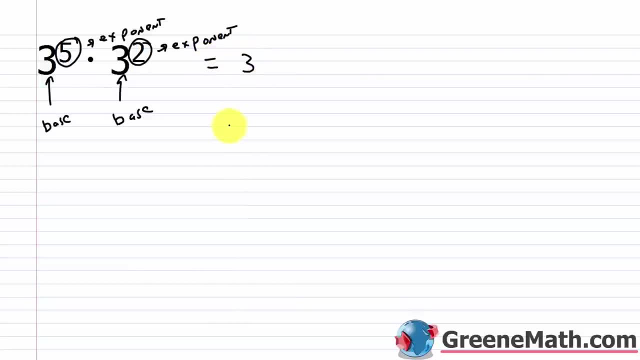 same. So just write a 3, and then I'm going to add the exponents, So I'm going to add 5 plus 2.. So it would be 3 raised to the power of 5 plus 2, which is 3 to the 7th power, And again one more time to get a complete. 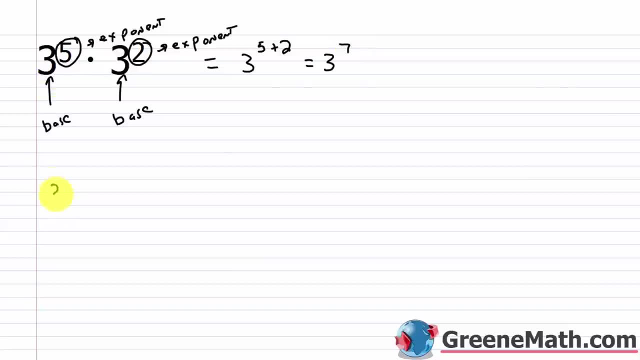 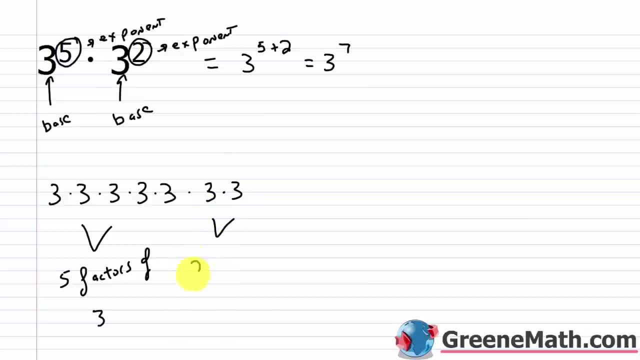 3 times 3.. So this would be 2 factors, 2 factors of 3.. So how many total factors of 3 do I have? Well, I have 7.. I have 5 factors here, plus I have 2 factors here, which is exactly what I did up here. So I have 3 raised to the power of 5 plus. 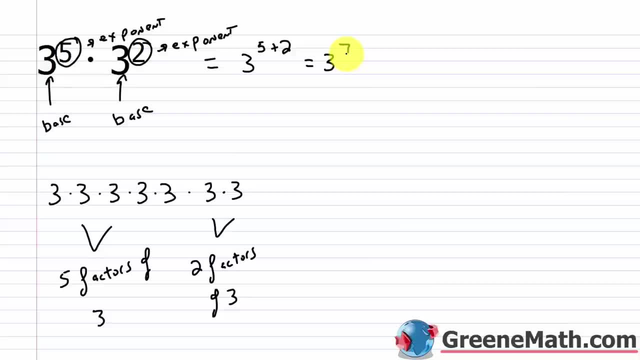 2, or 3 raised to the 7th power, And again you can go through and evaluate that if you want. but that's not really what we're trying to do. We're just trying to kind of simplify it and put 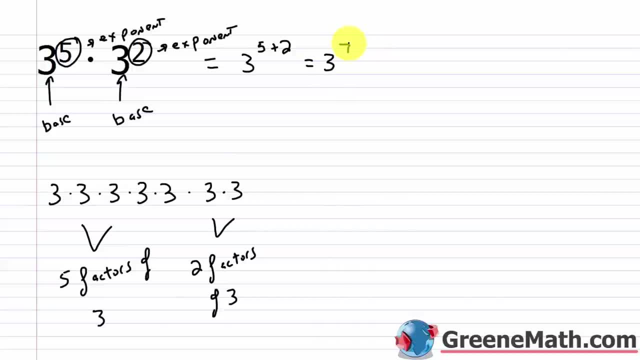 it in this form: Usually in your book they're not going to say, hey, evaluate 3 to the 7th power. They're just going to say: what is 3 to the 5th power, times 3 squared. Write that using an exponent right. So that's what. 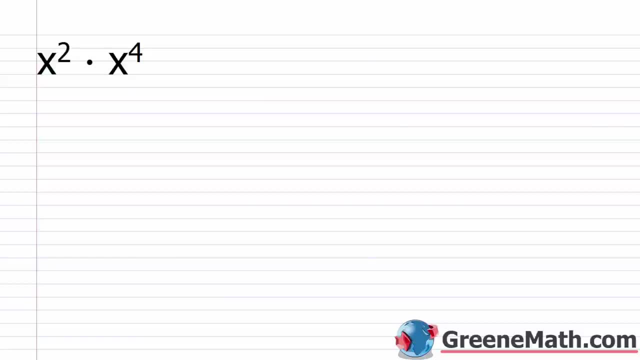 we've done. We have 3 to the 7th. All right, let's look at one with a variable. So we have x squared times x to the 4th power. So is there anything that's going to be different here? 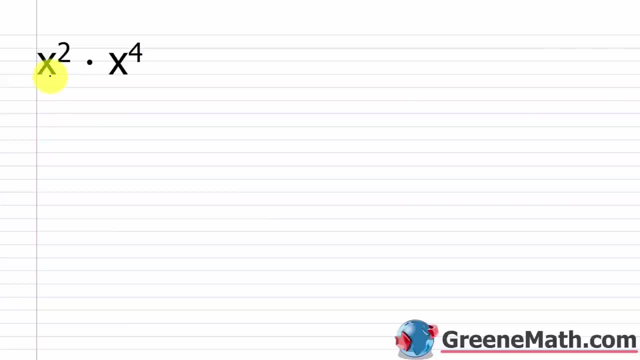 No, So I'm just going to do the same thing. I'm looking at the base. The base is the same. I have an x and I have an x. So when I do this multiplication, the base stays the same. I have x. So I'm just going to do the same thing. I'm looking at the base. I have an x and I have. 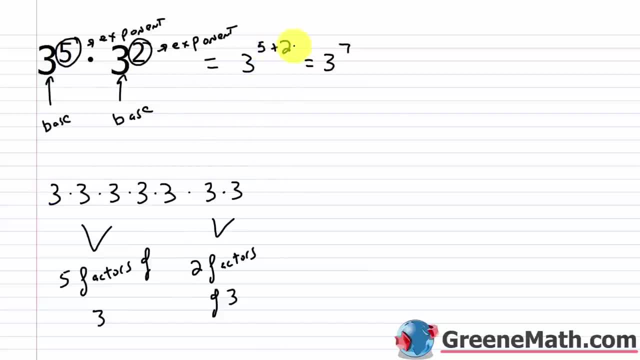 So I have three raised to the power of five plus two or three raised to the seventh power. And again you can go through and evaluate that if you want but that's not really what we're trying to do. We're just trying to kind of simplify it and put it in this form. Usually in your book they're not going to say hey evaluate three to the seventh power. They're just going to say what is three to the fifth power 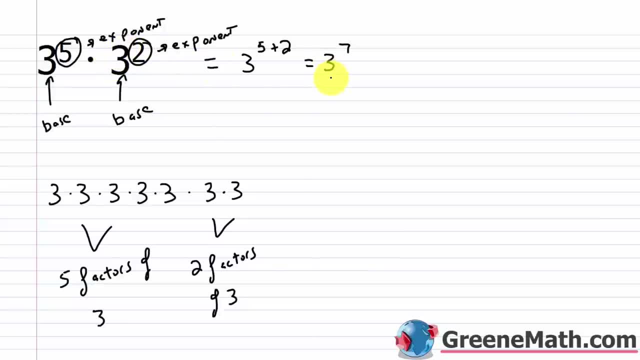 times three squared. Write that using an exponent. Right so that's what we've done. We have three to the seventh. All right let's look at one with a variable. So we have x squared times x to the fourth power. So is there anything that's going to be different here? No. So I'm just 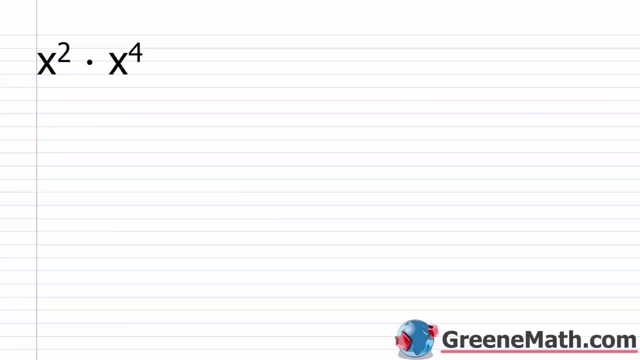 going to do the same thing. I'm looking at the base. The base is the same. I have an x and I have an x. So when I do this multiplication the base stays the same. I have x. And then I'm just going to add the exponents. I have a two here and a four here. So two plus four is six. So this is x to the sixth power. All right let's take a look at another one. We have z to the eighth power times z times 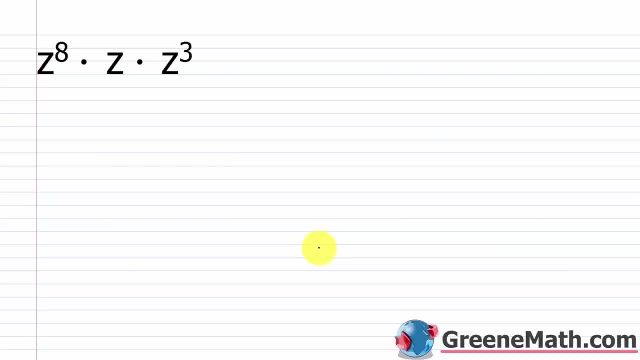 z cubed. So can we extend this to multiplication where now we have x squared times z cubed. So we're going to have three of these guys involved. Well yes we can. I know the original definition said a to the m times a to the n is equal to a to the power of m plus n. But it doesn't matter. I could go through and put z to the fourth times z to the ninth times z to the twelfth. I can keep going 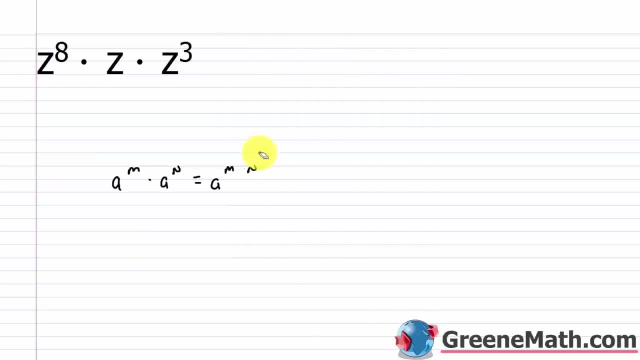 and going and going. As long as the base is the same. Okay as long as the base is the same there's so base is the same. I keep it the same. And then I just add the exponents. So I have an exponent here of eight. Then plus. Here I don't have a visible exponent. So what am I going to put? And 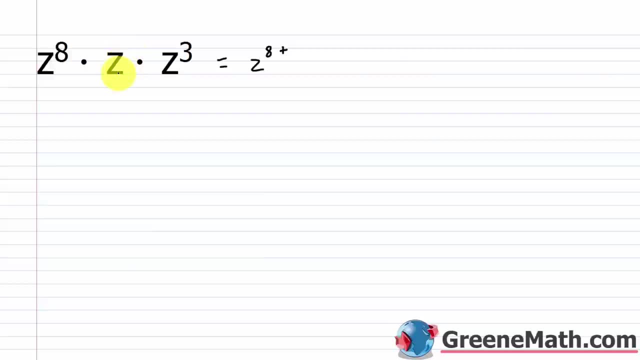 this is very very important. If you don't have a visible exponent the exponent is one. 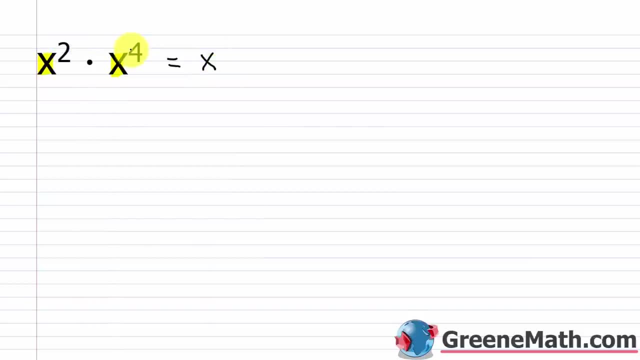 an x, And then I'm just going to add the exponents. I have a 2 here and a 4 here. So 2 plus 4 is 6.. So this is x to the 6th power. All right, let's take a look at another one. We have z to the 8th power. 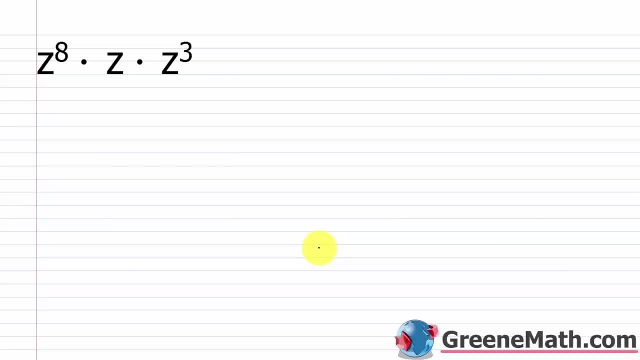 times z times z cubed. So can we extend this to multiplication, where now we have 3 of these guys involved? Well, yes, we can. I know the original definition said a to the m times a to the n is equal to a to the power of m plus n, But it doesn't matter. I could go through and put z to the 4th. 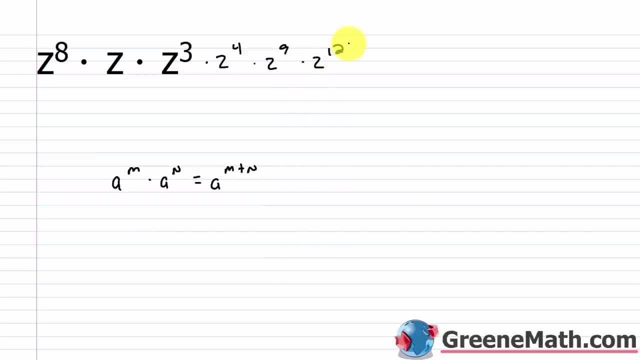 times z to the 9th, times z to the 12th. I can keep going and going and going. As long as the base is the same. there's really no limit. So base is the same, I keep it the same, And then I just add the. 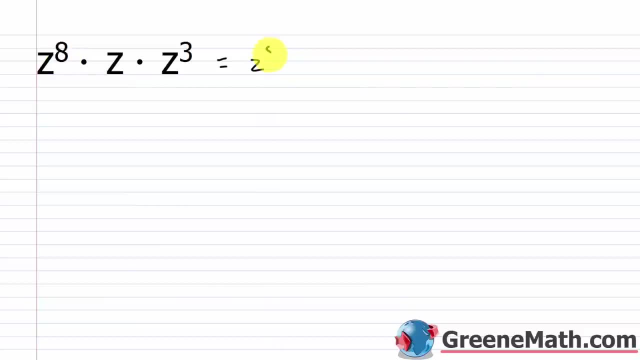 exponents. So I have an exponent here of 8, then plus Here I don't have a visible exponent. So what am I going to put? And this is very, very important- If you don't have a visible exponent? the exponent is 1. Because I have z to the 1st power there, or one single z, And it's very. 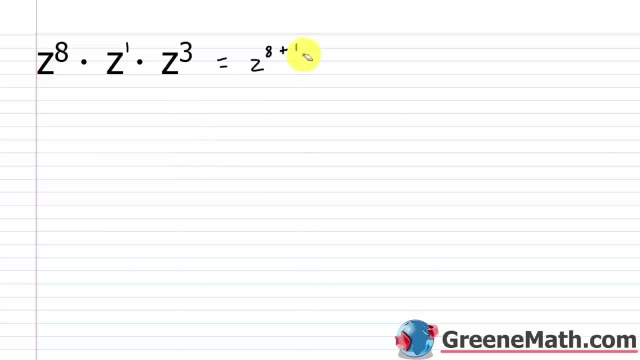 important that you put that, because some students will skip that over and just put 0 there. Well, you have to account for that factor of z in the end result. So if you put a 0 there, you will be 1 short. Now this one is z cubed, So I'm going to put plus. 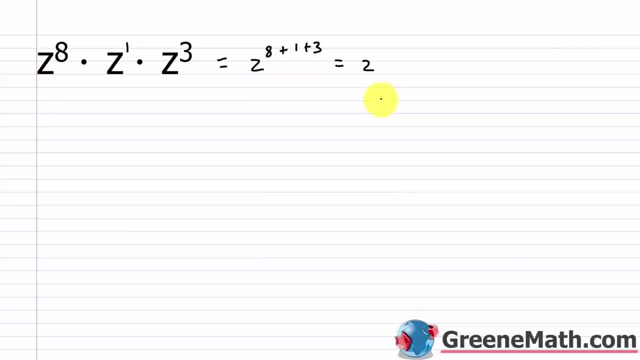 So then I would have z to the power of 8 plus 1 is 9,, then 9 plus 3 is 12.. And again, if you wanted to write that out and see that you would be short if you left this one off, go ahead and write out. 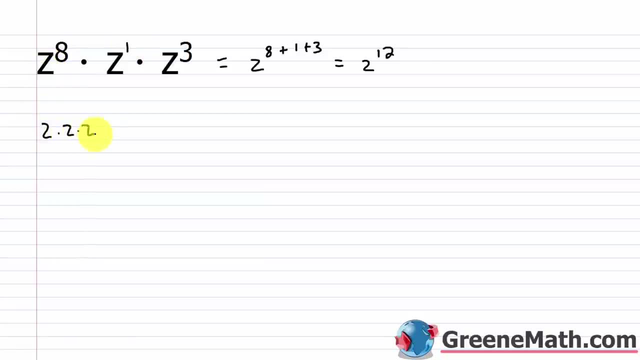 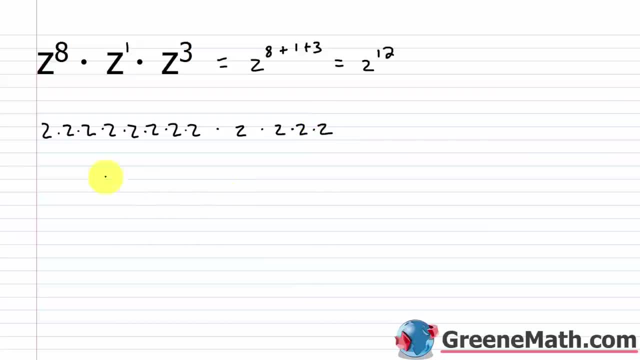 z times z times z. So as a total, you have 8 here, You have 1 here, And then you have 3 here. So that's 8 plus 1 plus 3, or 9 plus 3, which is 12.. If I had not counted this one, if I had said: 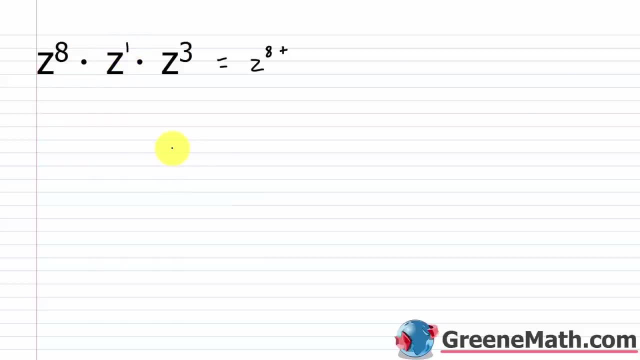 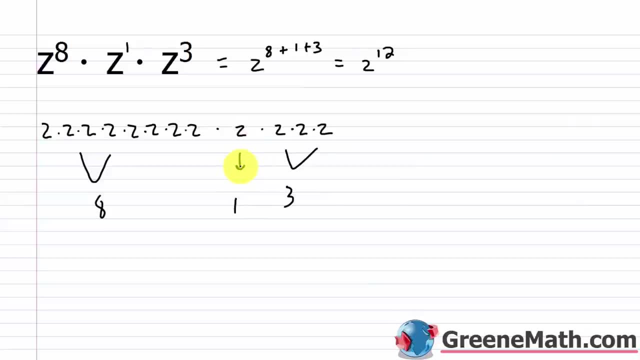 If I had not counted this one, if I had said, okay, well, there's no exponent there, so I'll leave it off, well, then you're not going to count this, and you're going to have 8 plus 3, which is 11, it's going to give you the wrong answer. So this is an understood exponent of 1. Make sure that if you come across that situation, you account for it. Okay, so the product rule for 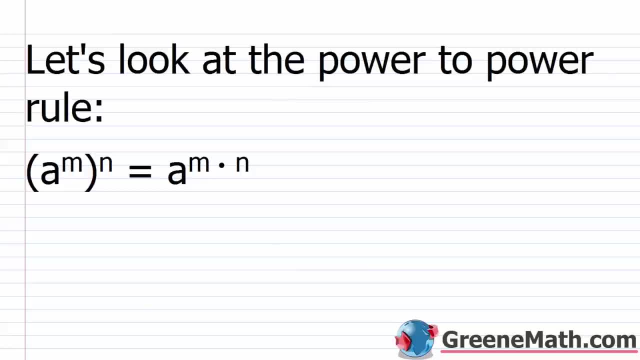 exponents, very, very simple, very, very easy to use. Just practice it, and you'll memorize it very, very quickly. So the next thing we want to look at are, 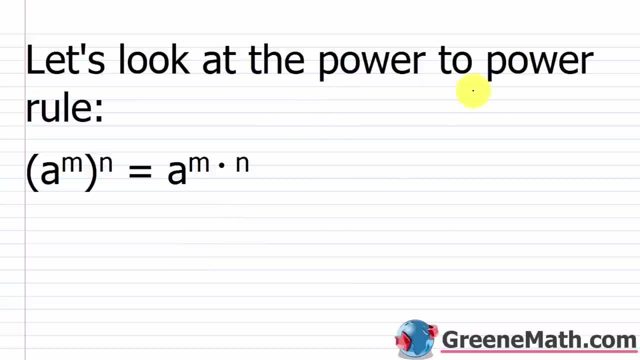 some power rules. And kind of the first one would be the power to power rule. So that's where you have something like a to the power of m. So a is already raised to something, and then you raise that whole thing to another power. So a to the power of m is now raised to the power of n. 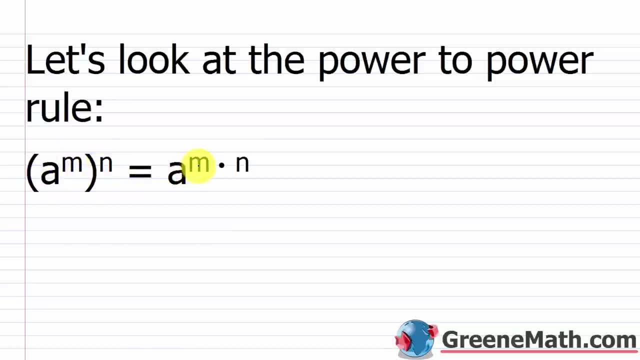 You can see this is equal to a raised to the power of m times n. So again, I don't like to give these textbook definitions, but essentially, you're just, 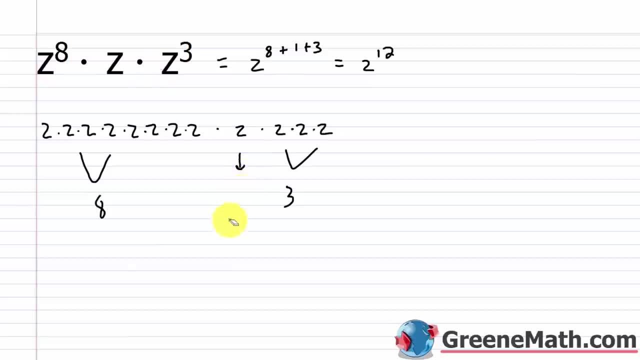 OK, well, there's no exponent there, So I'll leave it off. Well then, you're not going to count this And you're going to have 8 plus 3, which is 11.. It's going to give you the wrong answer. So this: 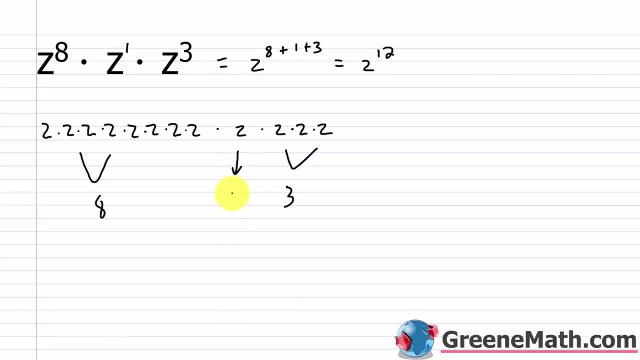 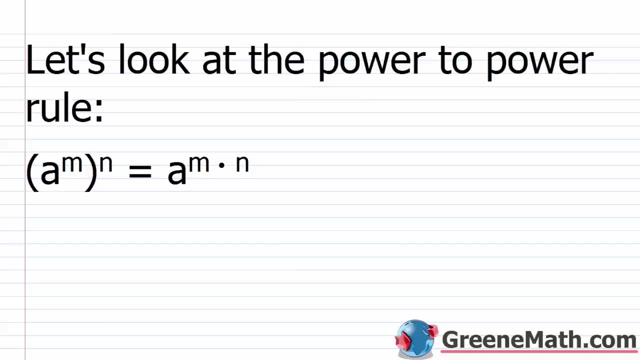 is an understood exponent of 1.. Make sure that if you come across that situation, you account for it. OK, so the product rule for exponents very, very simple, very, very easy to use. Just practice it and you'll memorize it very. 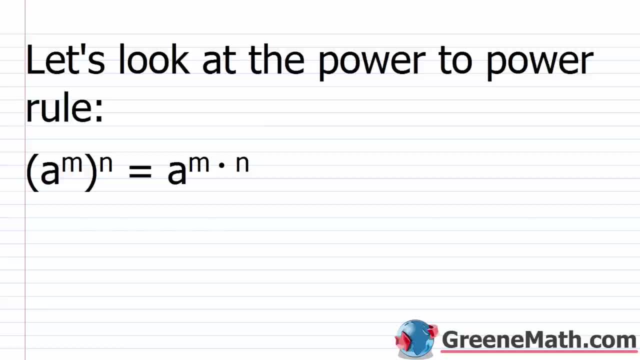 very quickly. So the next thing we want to look at are some power rules, And kind of the first one would be the power to power rule. So that's where you have something like a to the power of m, So a is already raised to something, And then you raise that whole thing to another power. So 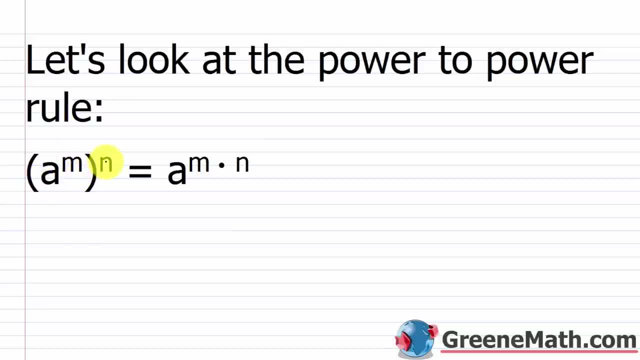 a to the power of m is going to be a to the power of m. So a to the power of m is going to be a to. the power of m is now raised to the power of n And you can see this is equal to a raised to the. 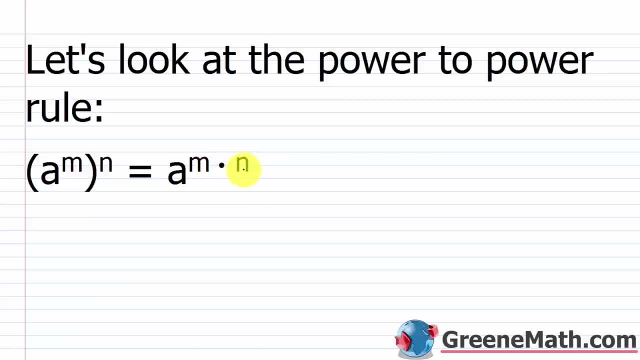 power of m times n. So again, I don't like to give these kind of textbook definitions, But essentially you're just keeping the base the same, So this original base stays the same, So that's the same. And then you're just multiplying the exponents, So something like: 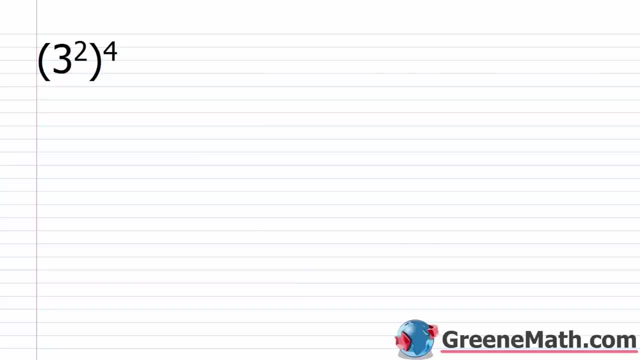 3 squared raised to the fourth power. Again, keep this original base 3 the same. So keep this the same And then just multiply the exponents, So I would have 2 times 4.. So 3 raised to the power of 2 times 4, which is 3 raised to the power of 8.. It's really really that simple. 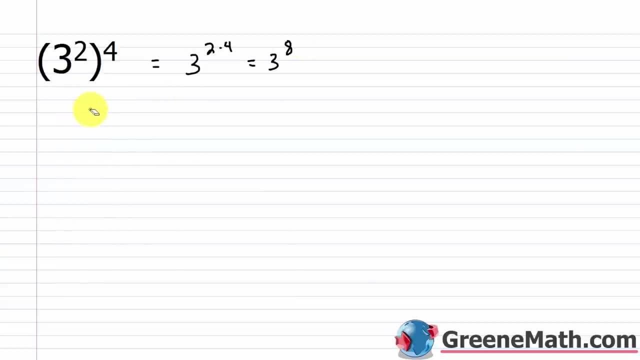 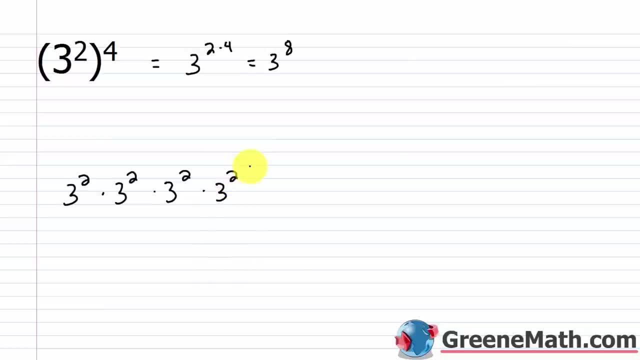 3 squared. So I already know from the product rule for exponents that we just learned. I would keep 3 the same and I would have 2 plus 2, which is 4 plus 2, which is 6 plus 2, which is 8.. So 3 to the. 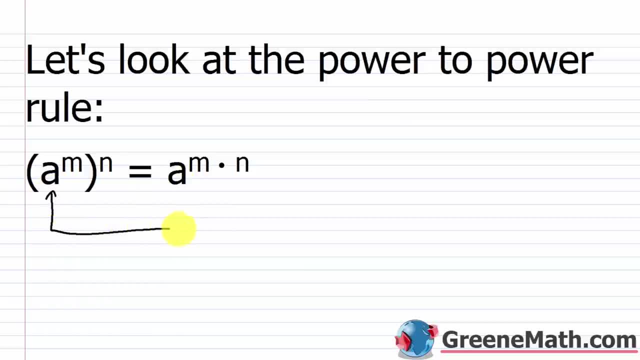 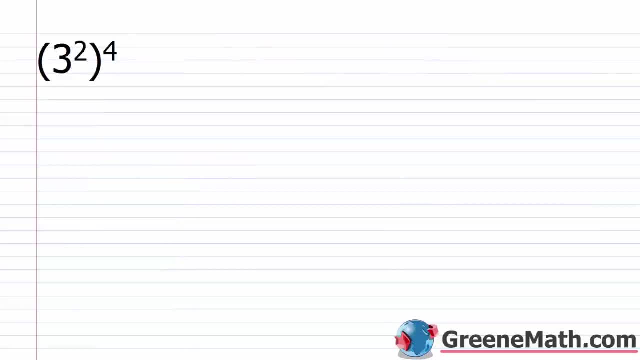 keeping the base the same. So this original base stays the same. So that's the same. And then you're just multiplying the exponents. So something like 3 squared raised to the fourth power. Again, keep this original base 3 the same. So keep this the same. And then just multiply the exponents. So 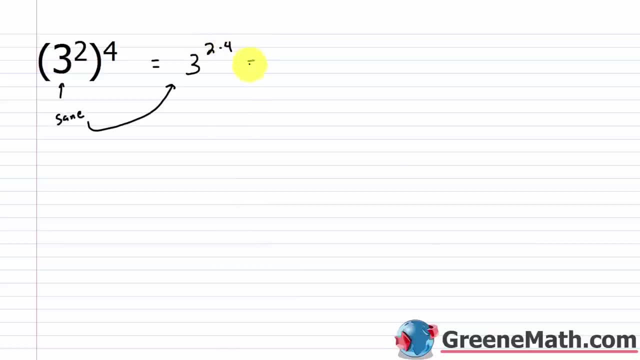 I would have 2 times 4. So 3 raised to the power of 2 times 4, which is 3 raised to the power of 8. It's really, really that simple. 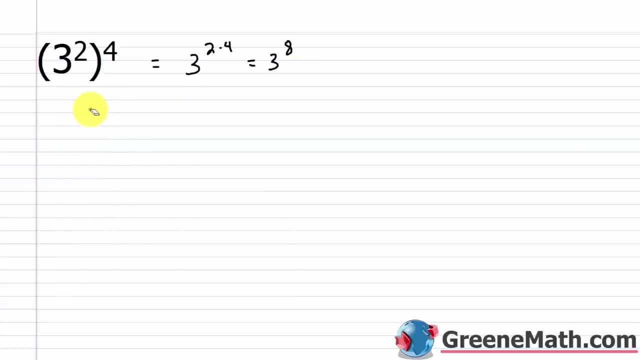 You can kind of think about why this works. 3 squared, 3 squared is being raised to the fourth power. So that means I'm going to have 4 of these. So times 3 squared, times 3 squared, times 3 squared. 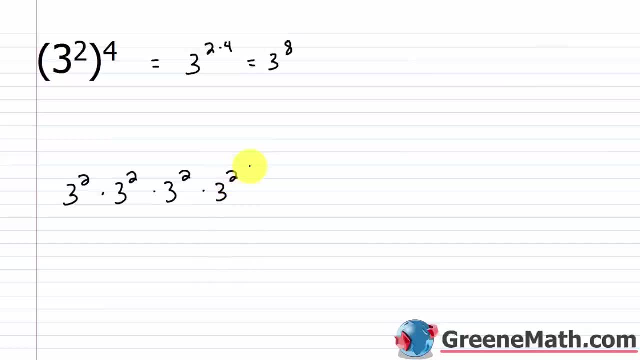 So I already know from the product rule for exponents that we just learned, I would keep 3 the same, and I would have 2 plus 2, which is 4, plus 2, which is 6, plus 2, which is 8. So 3 to the 8th power. But another way that you could think of about this is that this is going to happen 4 times. So if I have this many factors that's going to occur 4 times, I can just multiply. 2 times 4 would give me 8. That's kind of the shortcut. Because in the end, if I was to completely simplify this, I would end up with 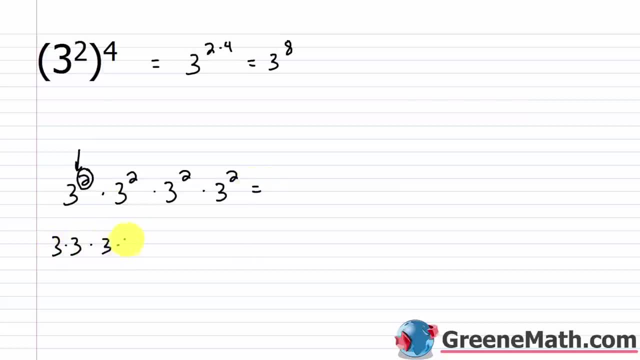 what? 2 factors of 3 times 2 factors of 3 times 2 factors of 3 times 2 factors of 3, or again, 3 to the 8th power. Let's take a look at 7 to the 5th power. 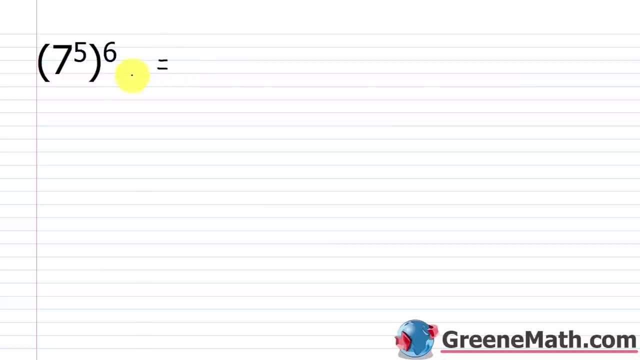 And then this is raised to the 6th power. So again, I'm just going to keep the base 7 the same, and multiply the exponents. So I multiply 5 times 6, and that's 30. So we get 7 to the 30th power. 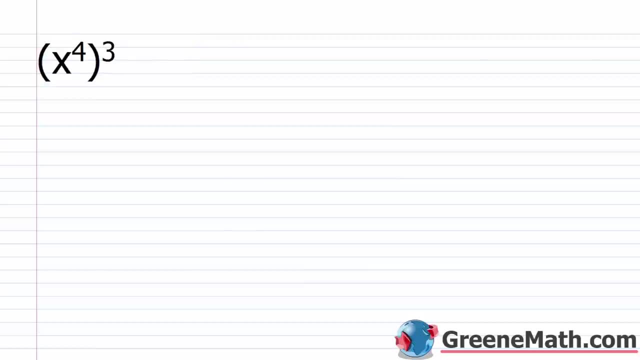 What about if we had a variable involved? Is anything going to be different? Well, no. If I have x to the 4th power, and then this is raised to the 3rd power, or cubed, I'm going to keep x the same. That's my base. And then I'm going to multiply. 4 times 3 is 12. 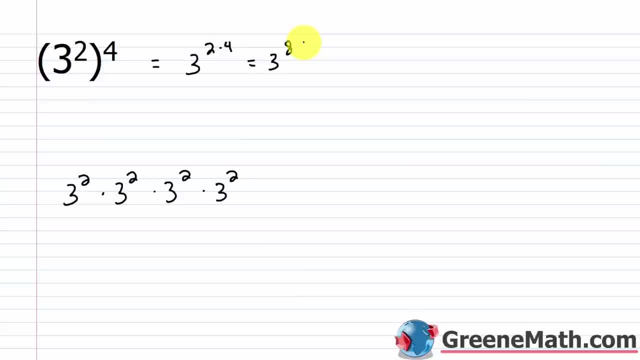 8th power. But another way that you could think about this is that this is going to happen four times. So if I have this many factors that's going to occur four times, I can just multiply 2 times 4 would give me 8.. That's kind of the shortcut, because in the end, if I was to completely simplify, 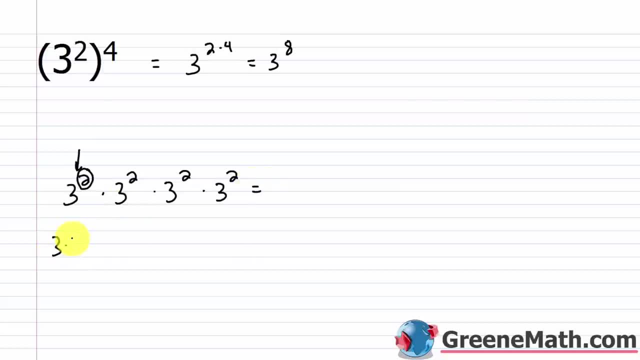 this. I would end up with what? 2? factors of 3 times 2, factors of 3 times 2, factors of 3 times 2, factors of 3, or again 3 to the 8th power. Let's take a look at 7 to the 5th power, and then this: 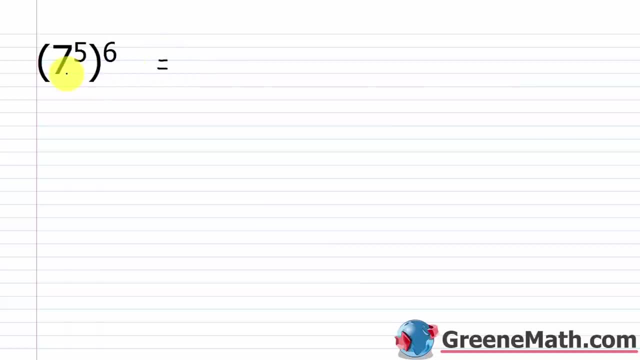 is raised to the 6th power. So again, I'm just going to keep the base 7 the same and multiply the exponents. So I multiply 5 times 6 and that's 30. So we get 7 to the 30th power. What about if? 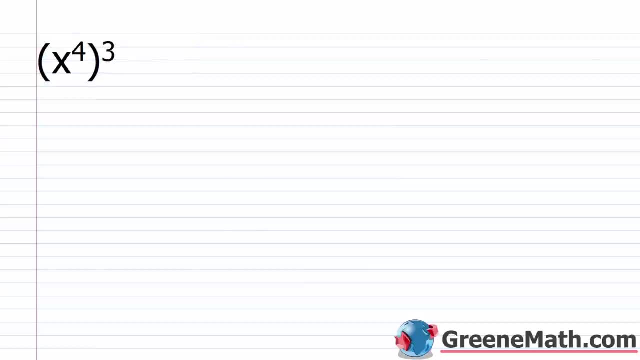 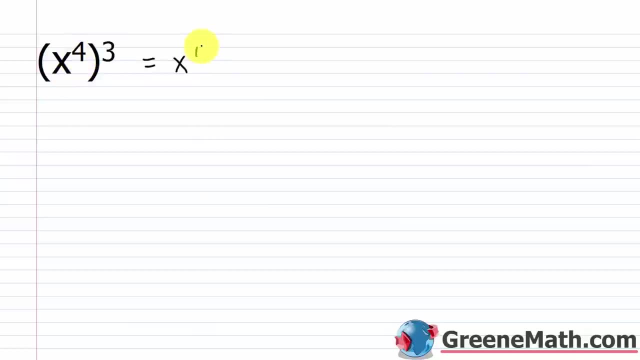 base and then I'm going to multiply 4 times 3 is 12.. So I would get x to the 12th power. What about z? raised to the 9th power, and then this is raised to the 8th power. Again, z is going to stay. 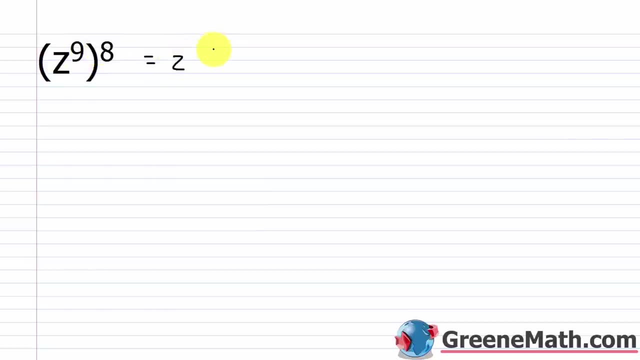 the same. Multiply the exponents 9 times 8 is 72.. What about y? to the 5th power, and then this whole thing is raised to the 3rd power Again. keep the base the same, So y is going to stay the same. Multiply the exponents 5 times 3 is 15.. Alright, 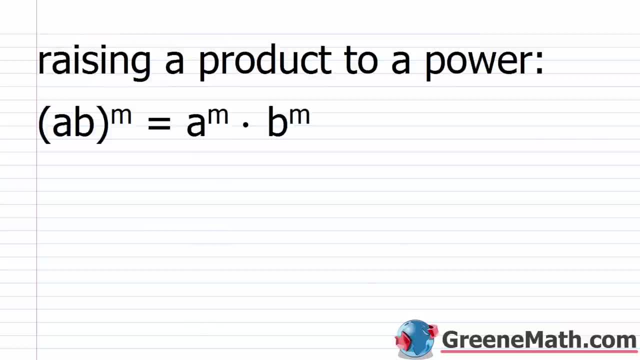 so continuing with the power rules. The next thing we want to talk about is raising a product to a power, And this one can go back and forth. So sometimes you'll need to simplify, You'll start out in this format and you need to go to this format. Sometimes you start out in this format. 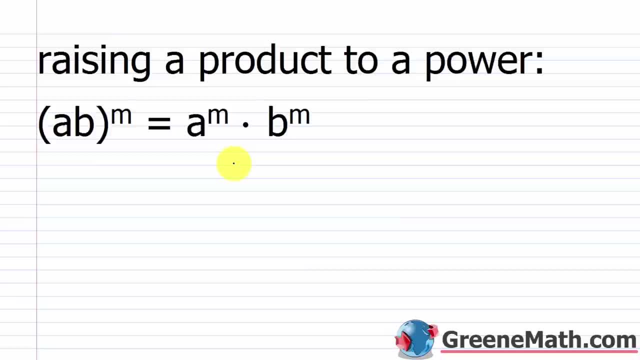 and you want to go to this format. Sometimes you want to go to this format, Sometimes you want to go back and forth between the two. It doesn't really matter. So if I have this product here which is a times b, So that product, and it's raised to the power of m, I can split it up and 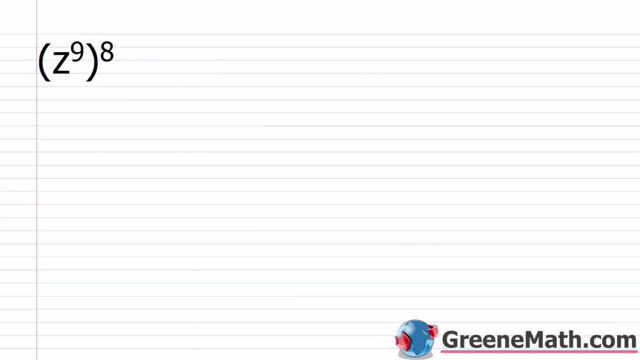 So I would get x to the 12th power. What about z raised to the 9th power? And then this is raised to the 8th power. Again, z is going to stay the same. Multiply the exponents. 9 times 8 is 72. 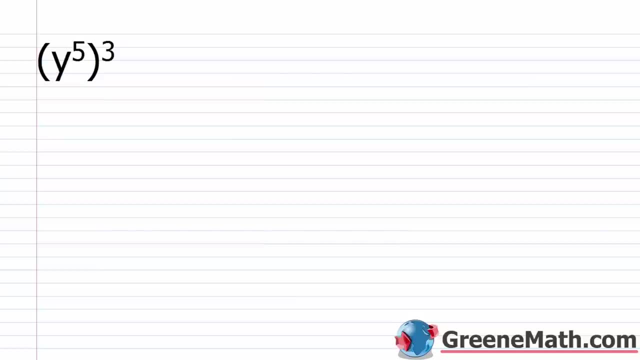 What about y to the 5th power? And then this whole thing is raised to the 3rd power. Again, keep the base the same. So y is going to stay the same. Multiply the exponents. 5 times 3 is 15. All right, so continuing with the power rules, the next thing we want to talk about is 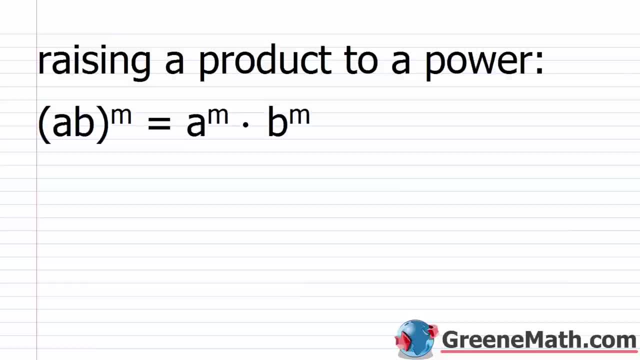 raising a product to a power. And this one can go back and forth. So sometimes you'll need to simplify. You'll start out in this format, and you need to go to this format. Sometimes you start out in this format, and you want to go to this format. You can go back and forth between the two. It doesn't really matter. So if I have this product here, which is a times b, so that product, and it's raised to the power of m, I can split it up and say this is equal to a to the power of m, 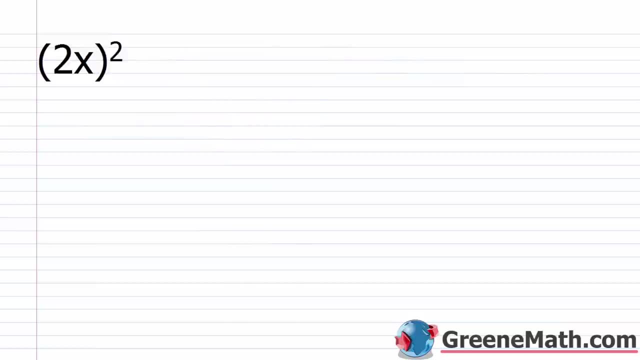 times b to the power of m. So in other words, if I have 2x, and this is raised to the power of 2, or it's squared, I can break this up and say that I have 2 squared times x squared, right? All I did 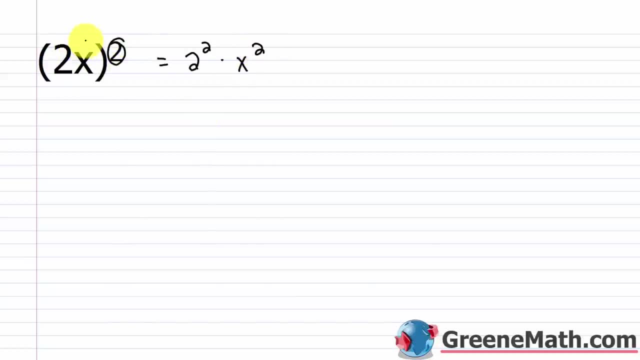 was take this and make it an exponent on each one of those individually. Now, I could further simplify this if I wanted to, because I know 2 squared is 4. So I could write this as 2 squared times x squared like that, or I could write it as 2 squared times x squared like that. That's 4x squared. And there's all kinds of manipulation that we're going to have to go through when we get to polynomials. It's just very important to know the rules so you know 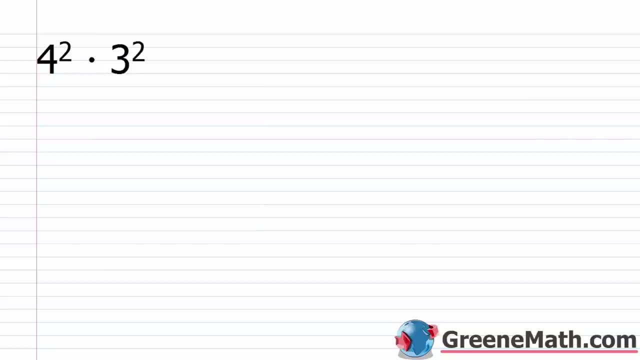 what's legal and what's not. So here we have an example of something that's presented a little differently. We have 4 squared times 3 squared. So to simplify this, if you get a problem, 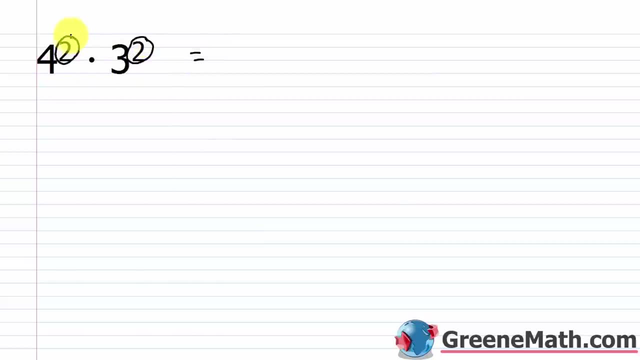 remember, I have the same exponent in each case. So what I can do is multiply the numbers or the bases together. So 4 times 3. 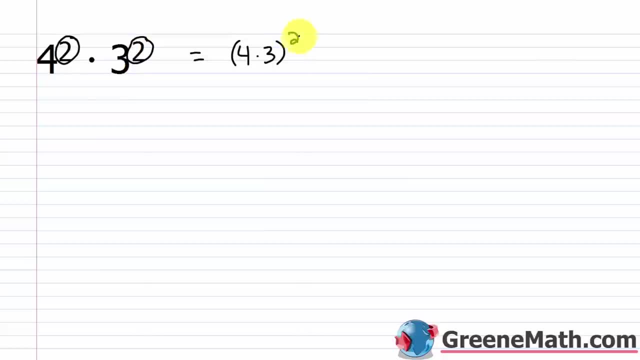 And then it's raised to that exponent that they each have, which is 2. So I have 4 times 3. That's going to be squared. And we know 4 times 3 is 12. So we could write this as 12 squared. So again, 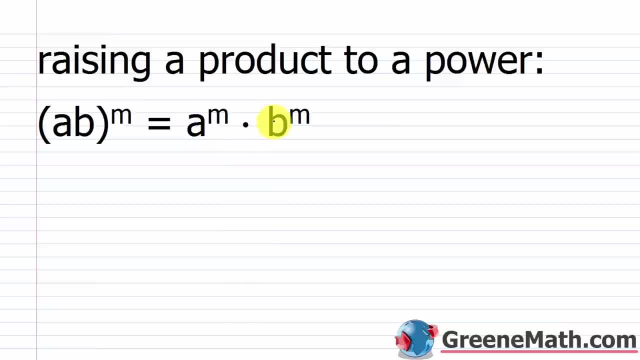 say this is equal to a to the power of m times b to the power of m. So in other words, if I have 2x and this is raised to the power of 2 or it's squared, I can break this up and say that I have. 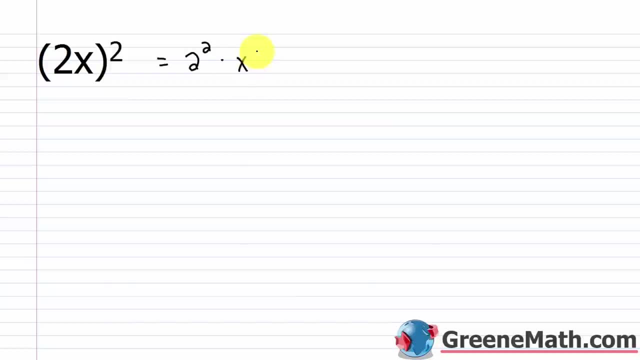 2 squared times x squared. Alright, all I did was take this and make it an exponent on each one of those individually. Now I could further simplify this if I wanted to, because I know 2 squared is 4. So I could write this as 2 squared times x squared, like that. Or I could write it as 4x squared. 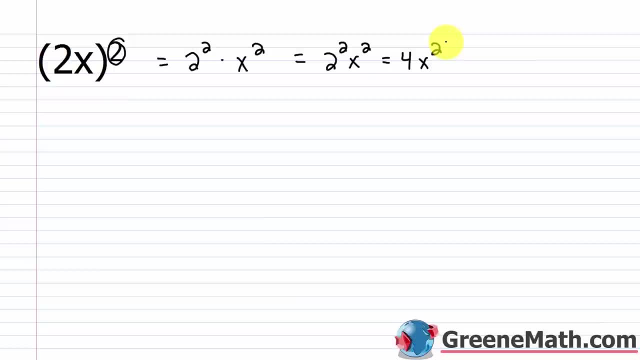 And there's all kinds of manipulation that we're going to have to go through when we get to polynomials. It's just very important to know the rules so you know what's legal and what's not. So here we have an example of something that's presented a little differently. 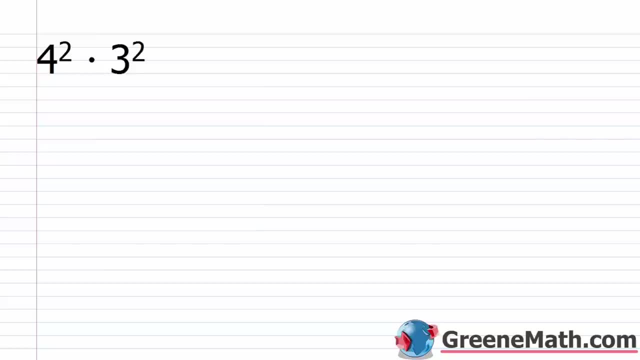 We have 4 squared times 3 squared. So to simplify this, if you get a problem, remember I have the same exponent in each case. So what I can do is multiply the numbers or the bases together, So 4 times 3, and then it's raised to that exponent that they each have, which is 2.. So I have 4 times. 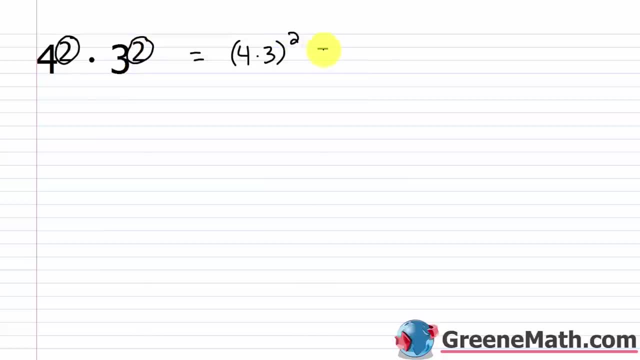 3.. That's going to be squared, and we know 4 times 3 is 12.. So we could write this as 12 squared. So again, just different ways to kind of simplify things. All right, what about 5xy? This is going to be raised to the 9th power. 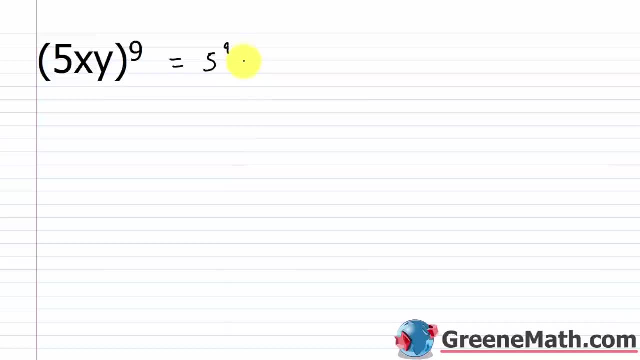 So we could simplify this and say we have 5 to the 9th power, times x to the 9th power, times y to the 9th power, So kind of separating this. each one is going to be raised to the 9th power, Or I. 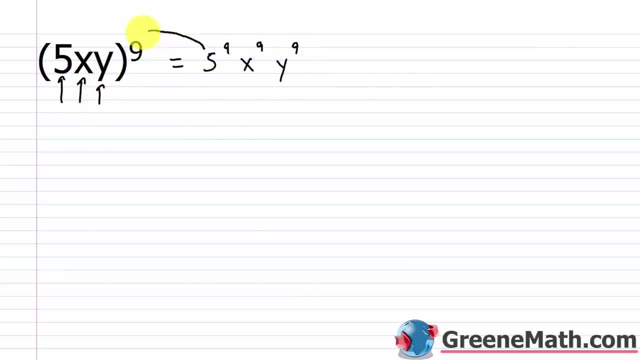 could go the other way. If I got this on a test, I could write it this way: where I have 5xy raised to the 9th power, because the exponent is the same in each case, What about 3z squared, 3zq raised to the second power or 3zq squared? Well, again, I can write this as 3 squared z squared. 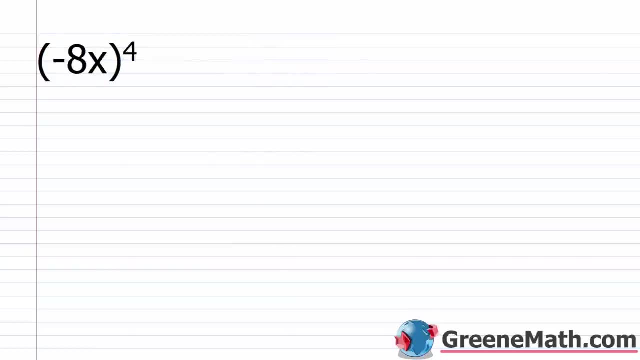 q squared. What about negative 8x to the 4th power? Well, one of the interesting things here is you have this negative out in front, So you can write this as you can write this as negative 8 to the 4th. 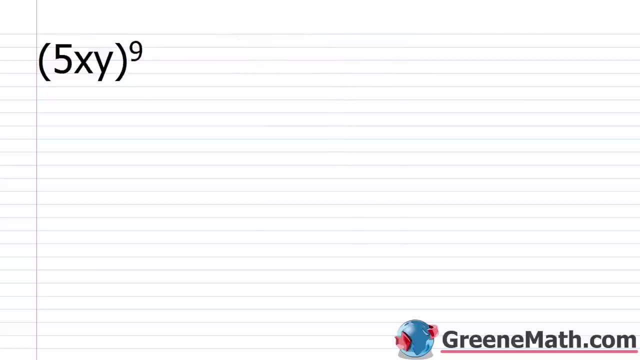 just different ways to kind of simplify things. All right, what about 5xy? This is going to be raised to the ninth power. So we could simplify this and say we have 5 to the ninth power times x to the ninth power times y to the ninth power. So kind of separating this, each one is going to be 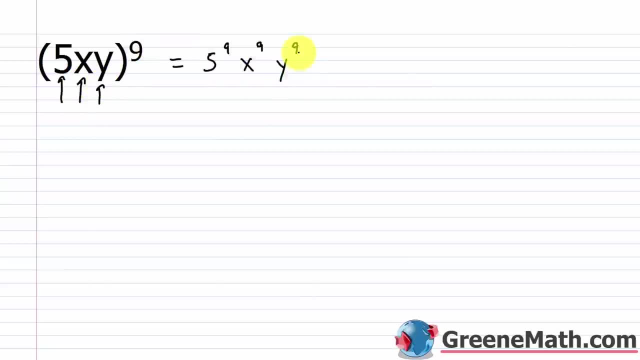 raised to the ninth power. Or I could go the other way. If I got this on a test, I could write it this way, where I have 5xy raised to the ninth power because the exponent is the same in each 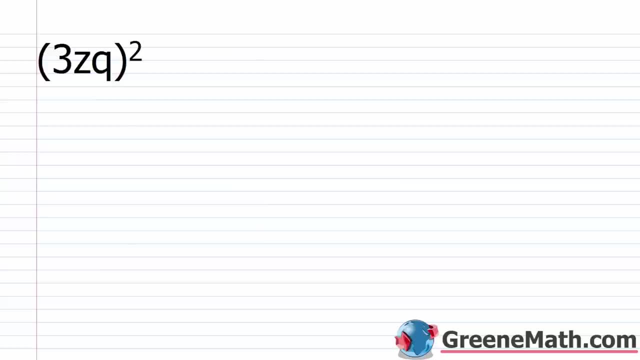 case. What about 3zq raised to the second power, or 3zq squared? Well, again, I can write this as 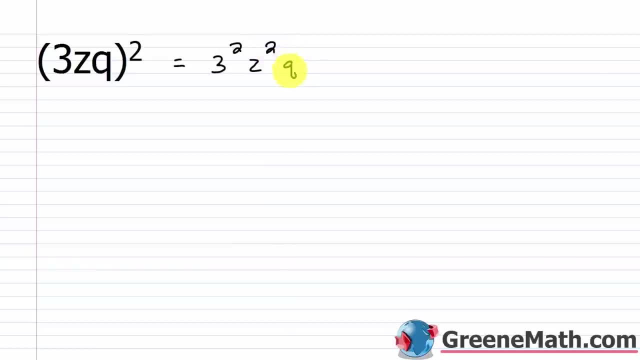 3 squared, z squared, q squared. What about negative 8x to the fourth power? Well, one of the interesting things here is you have this negative 8x to the fourth power, and you have negative out in front. So you can write this as negative 8 to the fourth power times x to the 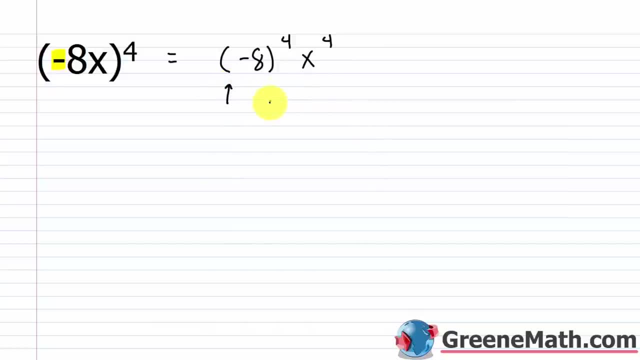 fourth power. Now notice how I use parentheses around that negative. That's highly, highly, highly important when you're working with exponents, particularly when you have an exponent that's even. Remember that from pre-algebra. If I have something like negative 2 squared, it's not going to be equal to negative 2 squared. It's going to be equal to negative 2 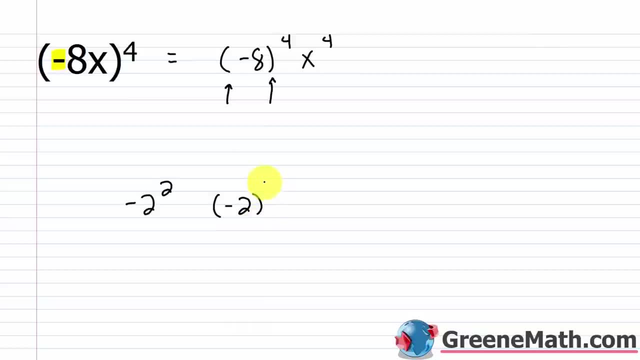 inside of parentheses squared. These two are not going to be equal. This right here is basically saying I have the opposite of 2 squared. So it's kind of like negative 1 times 2 squared, which is negative 1 times 4, or negative 4. If I have negative 2 inside of parentheses squared, this is saying I have negative 2 times negative 2, which equals positive 4. So pay close attention to that, especially when we get into algebra. 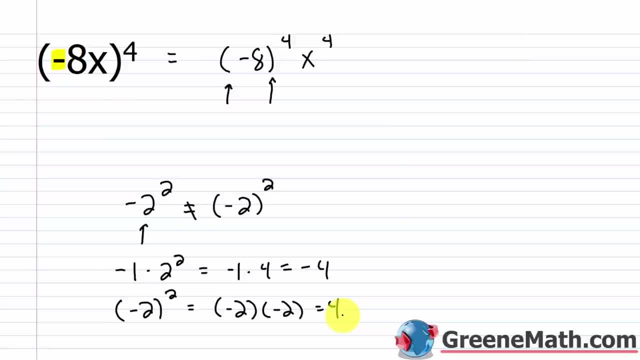 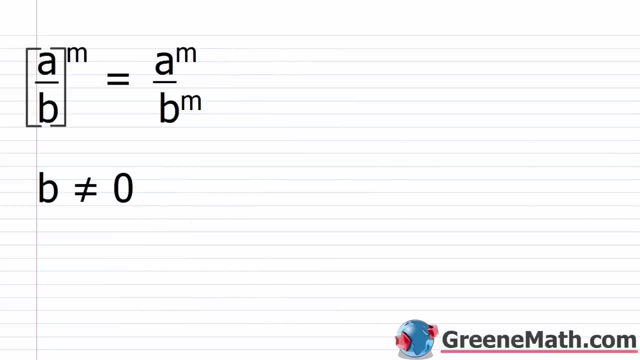 Because you're going to be expected to know this, and most teachers are not really going to cover that again. They expect you to kind of remember that from pre-algebra. All right, so let's take a look at our last power rule. So we have a over b. So you can think of this as a fraction or division. Remember, those are the same. This is a divided by b, however you want to think about it. 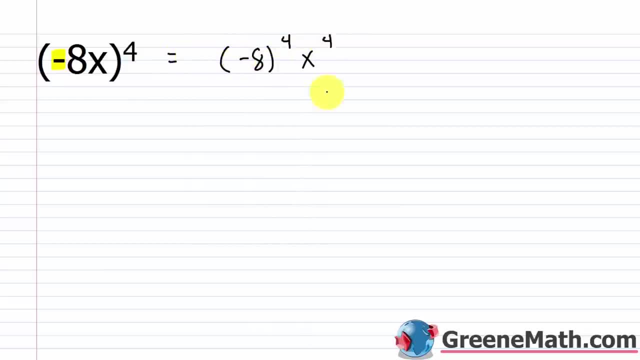 power times. x to the 4th power- I'm going to use parentheses around that negative. That's highly, highly, highly important when you're working with exponents, Particularly when you have an exponent that's even Remember that from pre-algebra, If I have something like negative 2 squared it's not going to be equal to negative 2. 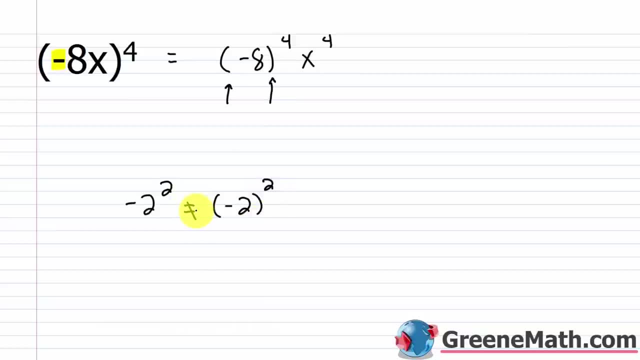 inside of parentheses squared, These two are not going to be equal. This right here is basically saying I have the opposite of 2 squared, So it's kind of like negative 1 times 2 squared, Which is negative 1 times 4 or negative 4.. If I have negative 2 inside of parentheses squared, this: 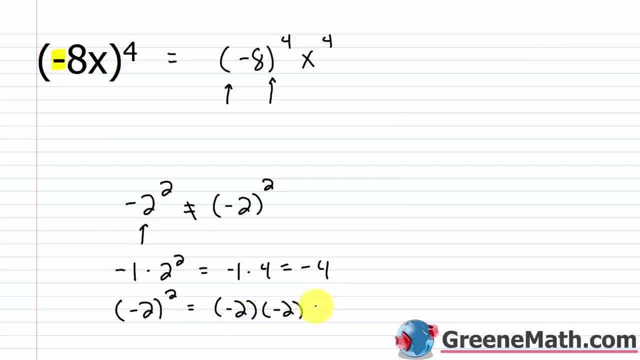 is saying I have negative 2 times negative 2, which equals positive 4.. So pay close attention to that, Especially when we get into algebra, because you're going to be expected to know this and most teachers are not really going to cover that again. They expect you to kind of remember that from. 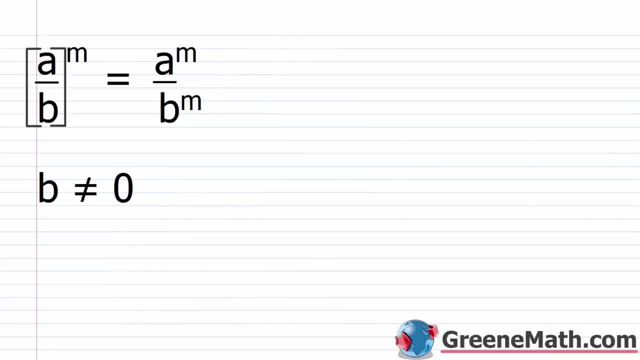 pre-algebra. All right, so let's take a look at our last power rule. So we have a over b, So you can think of this as a fraction or division. Remember, those are the same. This is a divided by b, however you want to think about it, And this is raised to the power of m. What we're saying is: 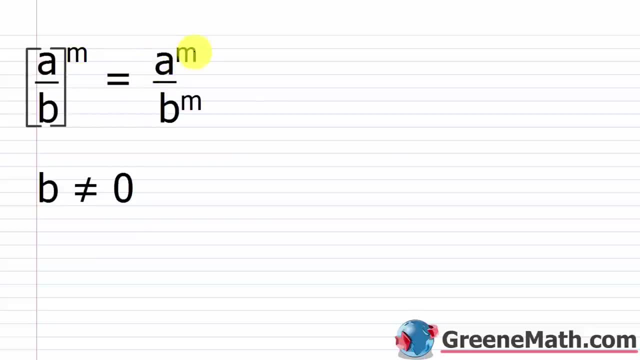 that this is equal to a, that numerator raised to the power of m, over b, that denominator raised to the power of m, And this again can go back and forth. Sometimes you'll need to write it this way. Sometimes you'll need to write it this way. One thing to note is that b cannot be 0. Why is that? 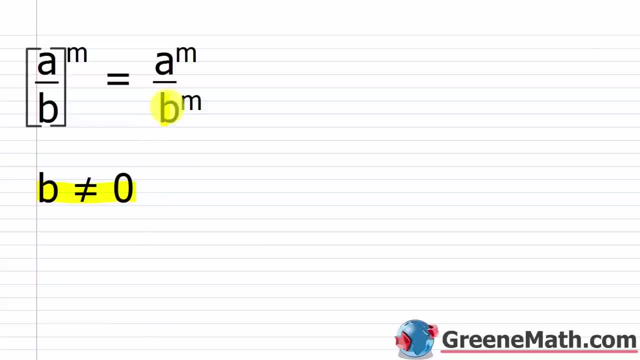 the case: B is in the denominator, B is in the denominator And we cannot divide by 0.. A is undefined, All right, so we have 8 over 4 and this is raised to the second power. So we could rewrite this as: 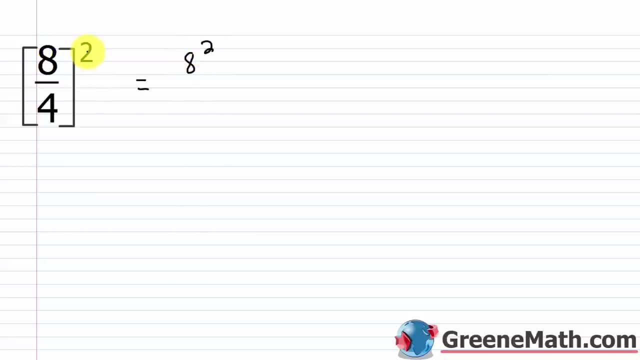 8 squared, Your numerator raised to that power. over 4 squared, Your denominator raised to that power, And there's all kinds of different things you can do to simplify this. You know, if you wanted to, you could have canceled this, with this to start and had 2.. 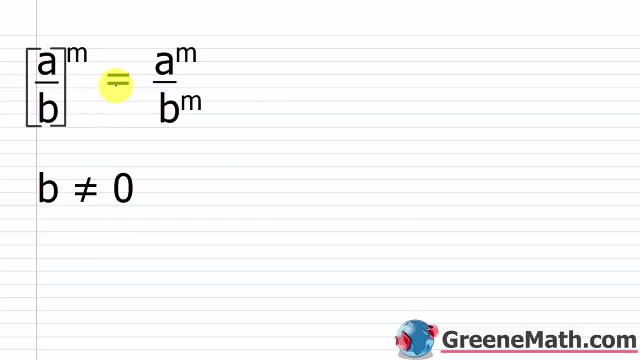 And this is raised to the power of m. What we're saying is that this is equal to a, that numerator raised to the power of m, over b, that denominator raised to the power of m, and this again can go back and forth. Sometimes you'll need to write it this way, sometimes you'll need to write it this way. But one thing to note is that b cannot be zero. Why is that the case? 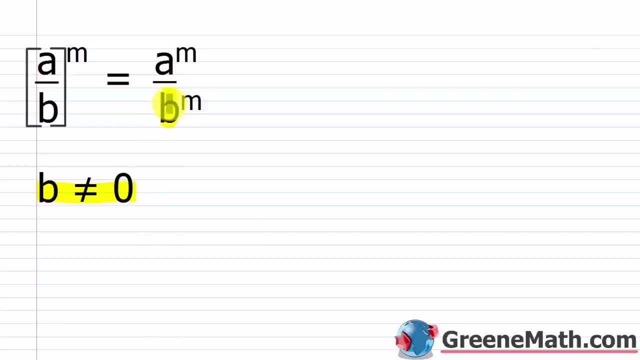 B is in the denominator. B is in the denominator, and we cannot divide by zero. A is undefined. All right, so we have 8 over 4, and this is raised to the second power. So we could rewrite this as 8 squared. 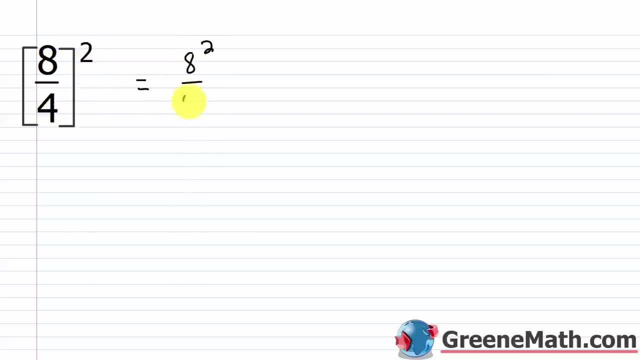 Over 4 squared, your denominator raised to that power. And there's all kinds of different things you can do to simplify this. You know, if you wanted to, you could have canceled this with this to start and had 2. So this is 2 squared of 4. But for the purposes of, you know, kind of learning this, this is how we're going to simplify for right now. And you can kind of go through and prove this to yourself. We know 8 over 4 would be 2, 2 squared is 4. So that's what this is equal to. 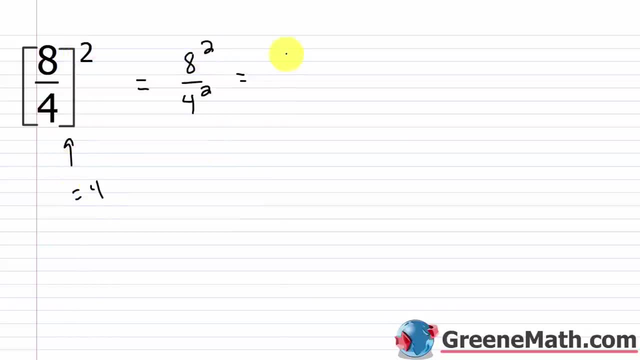 It's equal to 4. So here, 8 squared is 64. 4 squared is what? That's 16. Well, if I divide 64 by 16, I do get 4. 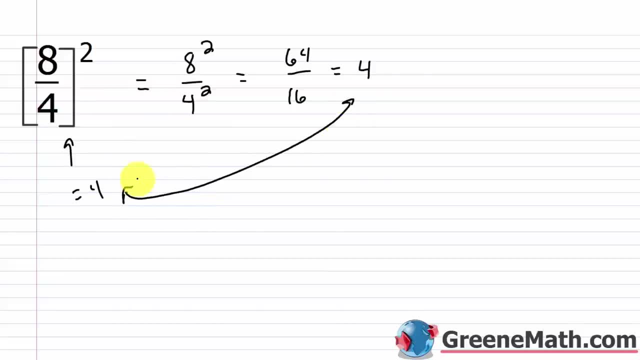 So it's the same either way. And of course, it should be. This should be mathematically equal to this. And when we go through and do the simplification in this matter, we get 4. We go through and do it the kind of original way where we divide 8 by 4 to start, then raise it to the second power, we also get 4. So again, it's the same either way. 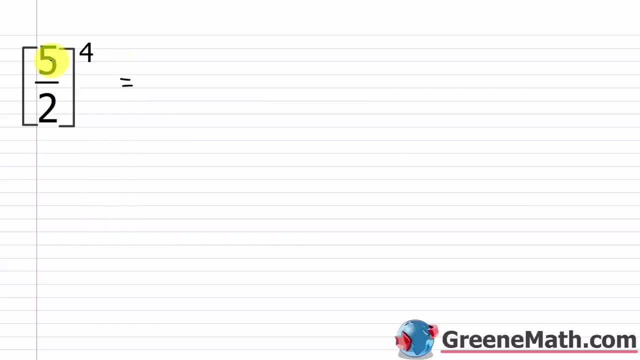 What about 5 halves raised to the fourth power? Well, again, I would just take 5, the number of the numerator, raise that to the fourth power, and put this over 2, the number of the denominator, raise that to the fourth power. What about x over y raised to the seventh power? Again, all I'm going to do is take x, that's what's in the numerator, and raise it to the seventh power, put this over y, which is in the denominator, and raise that in the seventh power. 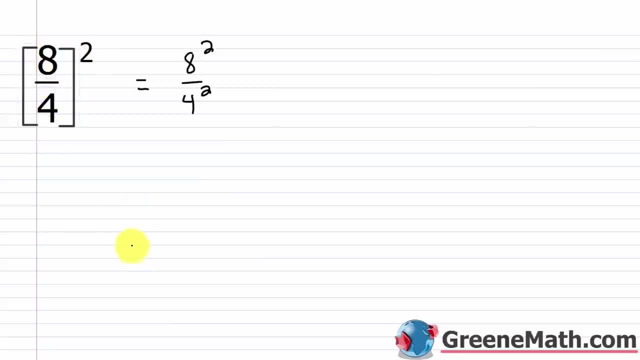 This is 2 squared or 4.. But for the purposes of you know, kind of learning this, this is how we're going to simplify for right now, And you can kind of go through and prove this to yourself. We know 8 over 4 would be 2.. 2 squared is 4.. So that's what this is equal to. It's equal to 4.. 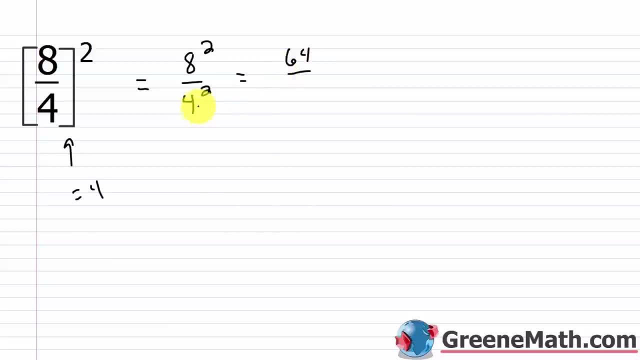 Over here, 8 squared is 64.. 4 squared is what, That's 16.. Well, if I divide 64 by 16, I do get 4.. So it's the same either way, And of course it should be. This should be mathematically equal to this, And when we go through and do, 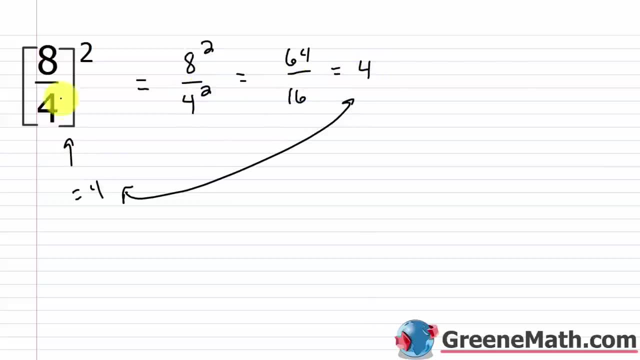 the simplification in this matter. we get 4.. We go through and do it the kind of original way where we divide 8 by 4 to start, Then raise it to the second power. We also get 4.. So again it's. 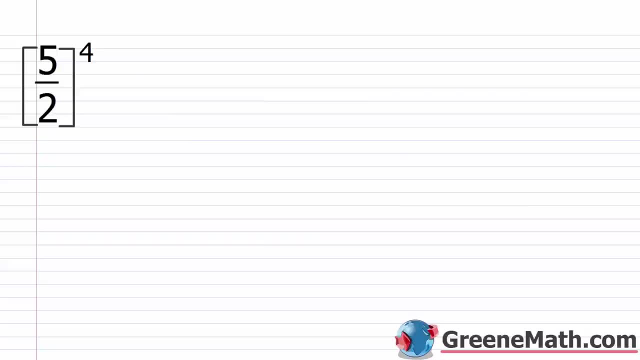 the same either way. What about 5 halves raised to the fourth power? Well, again, I would just take 5, the number of the numerator, Raise that to the fourth power And put this over to the number of the denominator. Raise that to the fourth power. 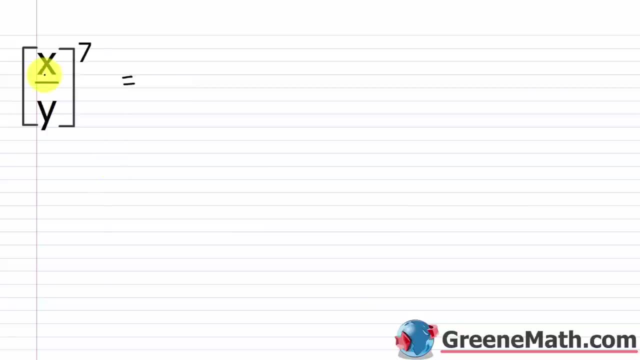 X over Y, raised to the seventh power. Again, all I'm going to do is take X- That's what's in the numerator, And raise it to the seventh power, Put this over Y, which is in the denominator, And raise that in the seventh power. Now, generally speaking, when we're working with variables, 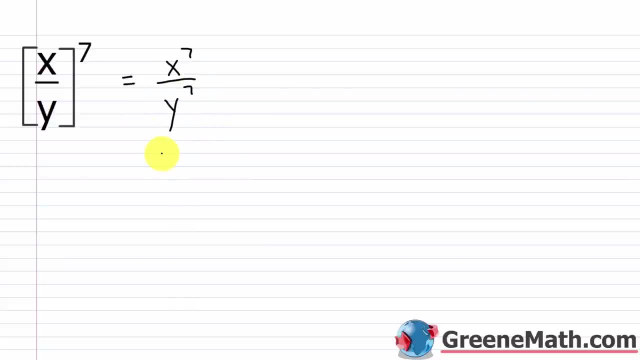 and we have a variable in our denominator. it's assumed that that variable in the denominator is not allowed to be 0 because that would be undefined. But you can specifically specify that Y is not equal to 0. Okay, but again, if you don't put that, it's logical to assume that that variable cannot be. 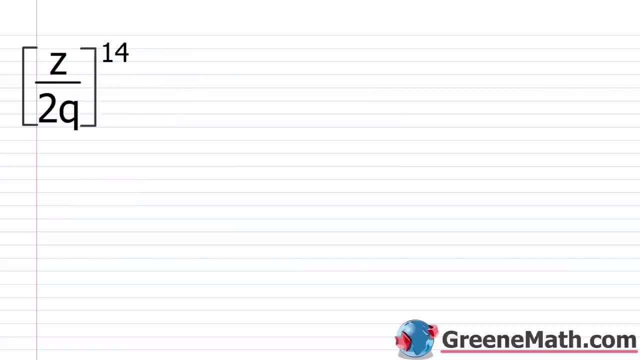 0.. All right, what about Z over 2q? and this is raised to the fourteenth power. So again, whatever's in the numerator, which is Z, that's raised to the fourteenth power, And this is over What's in the denominator. I have 2q, so the 2 would be raised to the power of. 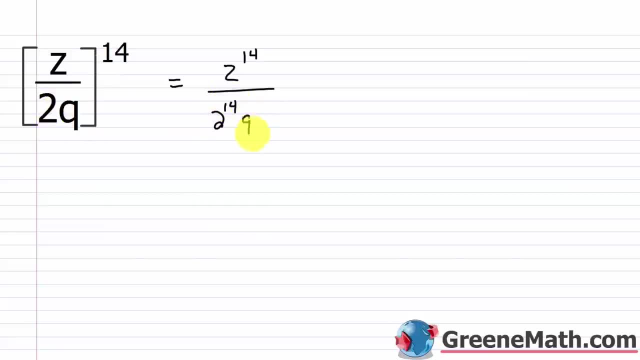 14, and so would the q. That would be raised to the power of 14 as well. You can kind of start out by thing: it will be a. You can kind of start out by thinking about it as: okay, this in the denominator, the 2q, is raised to the 14th power. 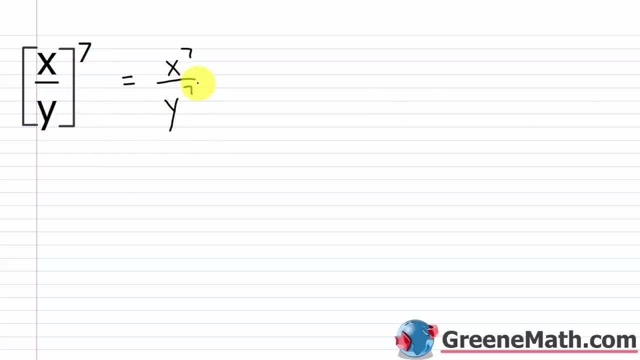 Now, generally speaking, when we're working with variables, and we have a variable in our denominator, it's assumed that that variable in the denominator is not allowed to be 0 because that would be undefined. But you can specifically specify that y is not equal to 0. But again, if you don't put that, it's logical to assume that that 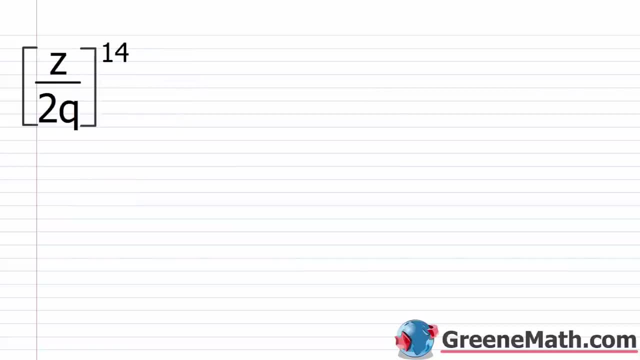 variable cannot be 0. What about z over 2q, and this is raised to the 14th power? So again, whatever's in the numerator, which is z, raised to the 14th power, and this is over, what's in the denominator? I have 2q. So the 2 would be raised to the power of 14, and so would the q. That would be raised to the power of 14 as well. You can kind of start out by thinking about it as, okay, this in the denominator, the 2q, 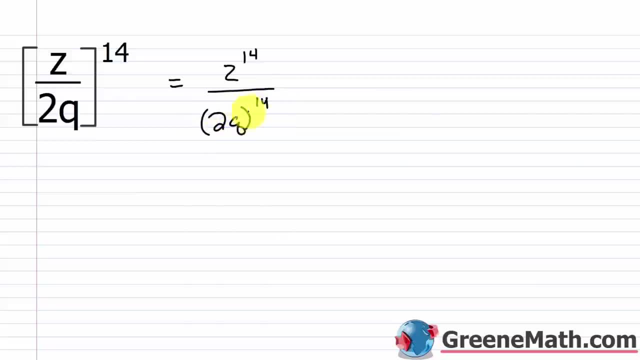 is raised to the 14th power. We've already learned that if we have that, we can kind of separate the 2 and the q and raise each to the 14th power. So again, we can just keep writing this as 2 to the 14th power times q to the 14th power. 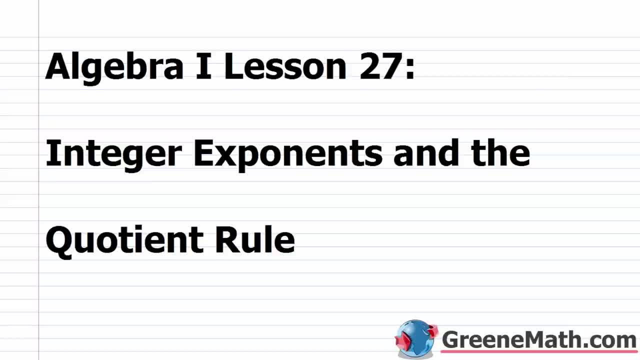 Hello and welcome to Algebra 1, Lesson 27. In this video, we're going to learn about integer 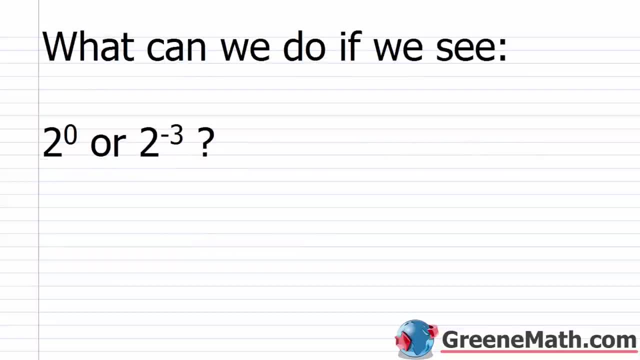 exponents and the quotient rule. So in our last lesson, we learned about the power rules for exponents, and we also talked about the product rule for exponents. Now we're going to expand on this and start to learn about negative exponents, the power of 0, and then the quotient rule for exponents. 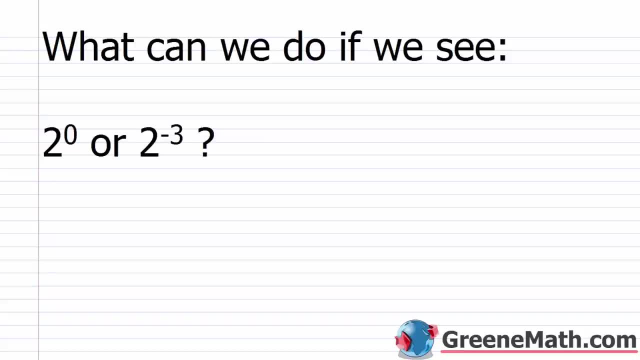 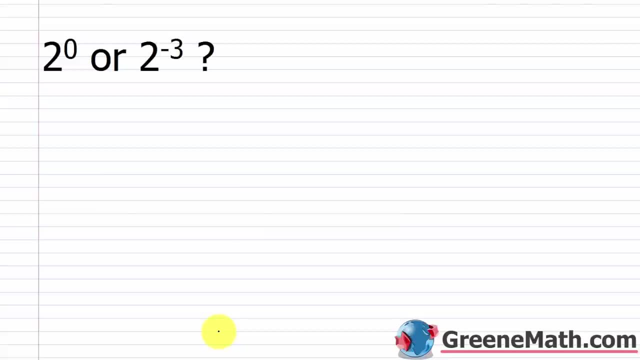 So I want to start today's lesson out by just asking a simple question. What can we do if we see something like 2 to the power of 0 or 2 to the power of negative 3? If I have something like 2 to the 4th power, I know that this is 4 factors of 2. 2 times 2 is 4, 4 times 2 is 8, 8 times 2 is 16. Then if I decrease the exponent by 1 and I have 2 to the 3rd power, now I have only 3 factors of 2, that's 8. If I have 2 squared, again if I decrease the exponent by 1, I have only 2 factors of 2, or 4. And then I know that if I just have the number 2, that has an exponent that's understood to be 1, so that's just the number 2. 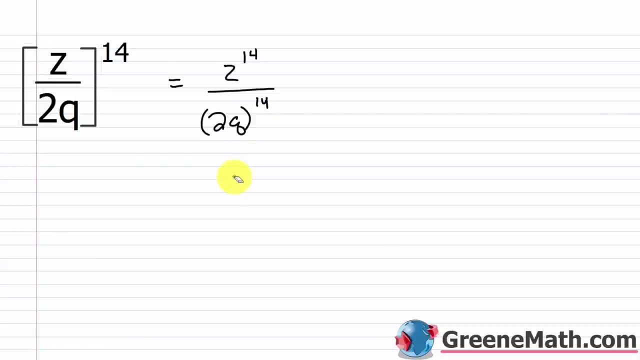 We've already learned that if we have that we can kind of separate the 2 and the q and raise each to the 14th power. So again, we end up writing this as: 2 to the 14th power, times q to the 14th power. 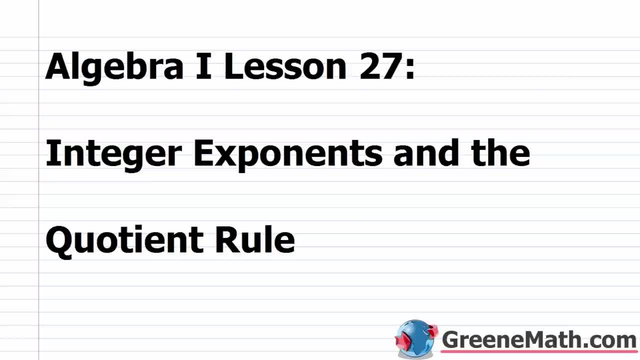 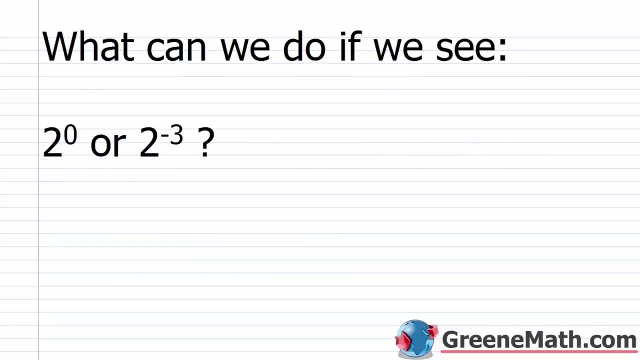 Hello and welcome to Algebra 1, Lesson 27.. In this video we're going to learn about integer exponents and the quotient rule. So in our last lesson we learned about the power rules for exponents and we also talked about the product rule for exponents. 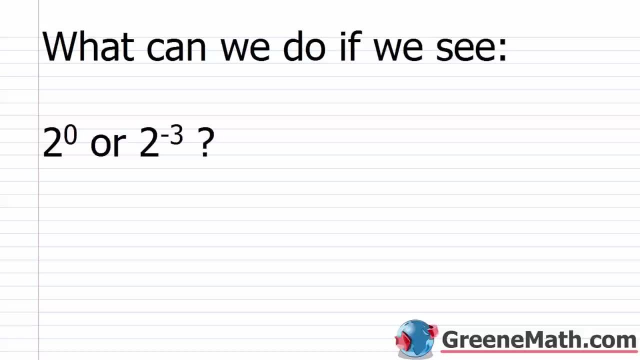 Now we're going to expand on this and start to learn about negative exponents, the power of 0, and then the quotient rule for exponents. So I want to start today's lesson out by just asking a simple question: What can we do if we see something like 2 to the power of 0 or 2 to the power of negative 3?? 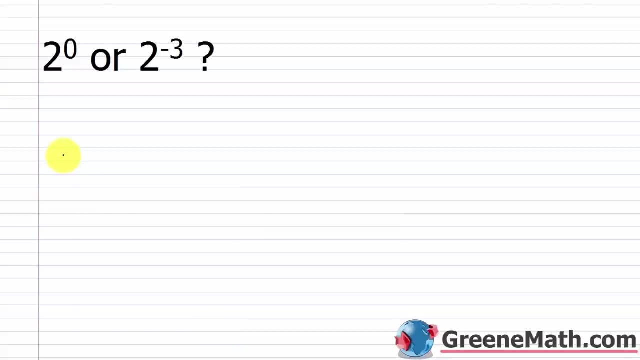 If I have something like 2 to the 4th power, I know that this is 4 factors of 2.. 2 times 2 is 4,, 4 times 2 is 8,, 8 times 2 is 16.. 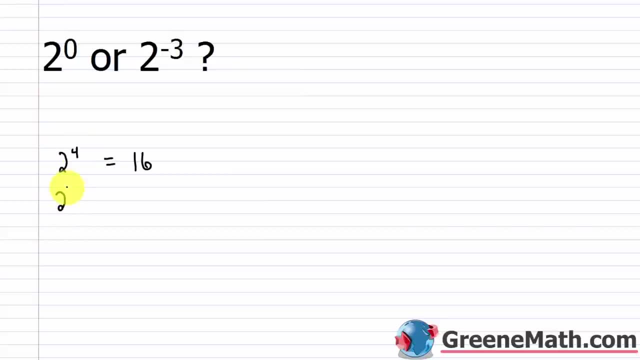 Then if I decrease the exponent by 1, and I have 2 to the 3rd power now I have 3 factors of 2, that's 8.. If I have 2 squared again, if I decrease the exponent by 1, I have only 2 factors of 2,. 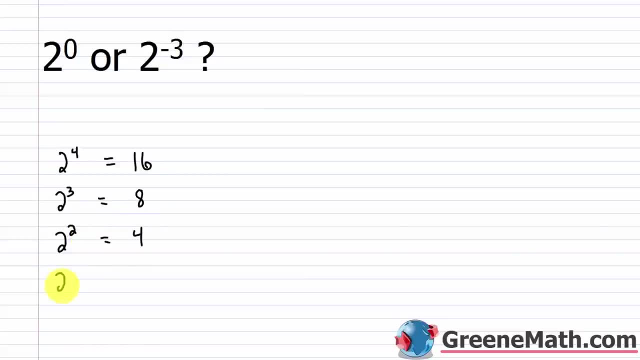 or 4.. And then If I have a number 2, that has an exponent that's understood to be 1, so that's just the number 2.. So now I'm going to put 2 to the power of 0 here, and I'm just going to put question. 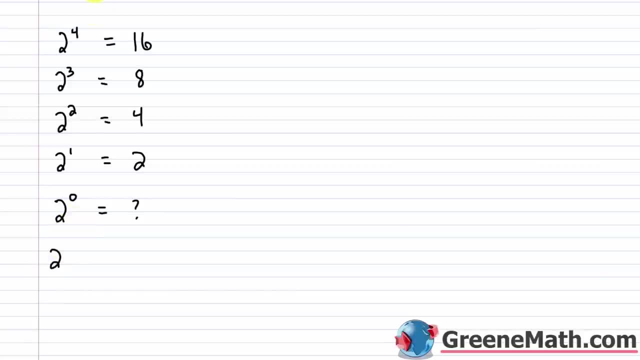 mark for right now. I'm also going to put 2 to the power of negative 1, and I'm going to put 2 to the power of negative 2.. And let's see if we can use some basic reasoning to get some answers here. 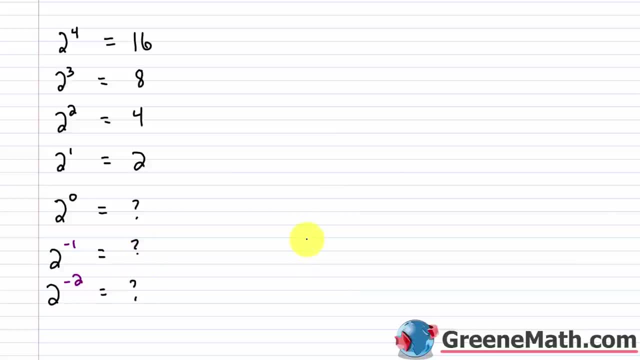 So the first question I would ask you is: do you notice any pattern here? Well, every time we increase our exponent by 1, you will notice that we take the result from the previous part and we multiply it by 2.. So, in other words, to get the answer for 2 squared. if I didn't know it, I can just take: 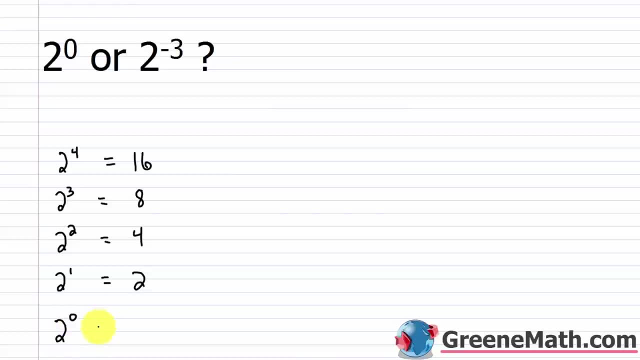 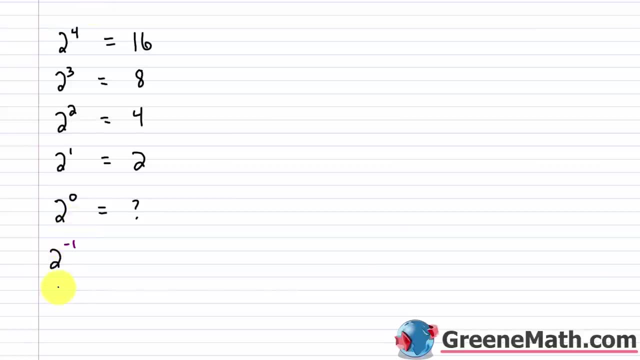 So now I'm going to put 2 to the power of 0 here, and I'm just going to put question mark for right now. I'm also going to put 2 to the power of negative 1. And I'm going to put 2 to the power 2 of negative 2. And let's see if we can use some basic reasoning to get some answers here. So the first question I would ask you is do you notice any pattern here? Well every time we increase our exponent by 1 you will notice that we take the result from the previous part and we multiply it by 2. So in other words to get the answer for 2 squared if I didn't know it I could just take the result from 2 to the first power and I could multiply it by another factor of 2 and I would get the result for 2 squared. So that would give me 4. What I could do again since I'm increasing my exponent by 1 I could just take this result which is 4 and multiply it by another factor of 2. That would give me 8. Again if I go up 1 in terms of my exponent I go to 2 to the fourth power. If I don't know what that is I can just take 8 which is the result from the previous one. 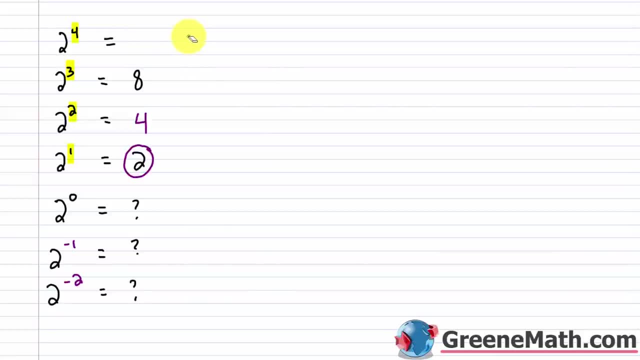 And again multiply it by 2. 8 times 2 is 16. Now that's obvious because each time I increase my exponent by 1 I'm basically taking the previous answer and I'm multiplying by another factor of 2. What happens if I go down though? Now I'm going to be dividing right the opposite of multiplication is division. So in other words let me kind of erase this real quick. If I start out at 2 to the fourth power the exponent is 4. If I go down to 2 squared I'm going to get 2 to the fourth power. If I go down to 2 to the fourth power the exponent is 4. If I go down to 2 to the fourth power the exponent is 4. If I go down to 2 to the fourth power the exponent is 4. If I go down to 2 to the third power I've decreased my exponent by 1. So if I didn't know what any of these were I could just start with 16 and say okay well I have 16 here I would just divide by 2. I'm just going to end up with the number 8 because essentially what I'm doing is I'm saying okay I had 2 to the fourth power which is 2 times 2 times 2 times 2 and now I'm going to remove a factor of 2 because I'm decreasing my exponent by 1. 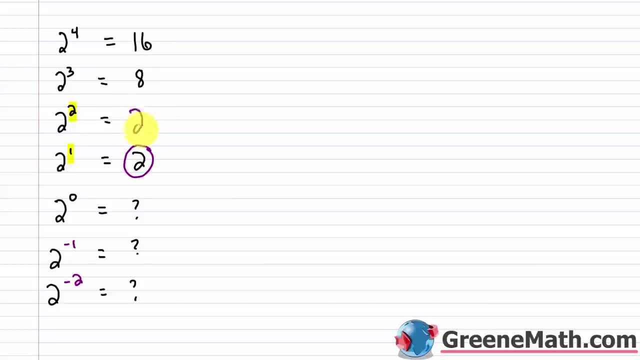 the result from 2 to the first power and I can multiply it by another factor of 2, and I would get the result for 2 squared, so that would give me 4.. What I could do again, since I'm increasing my exponent by 1,, I could just take this result. 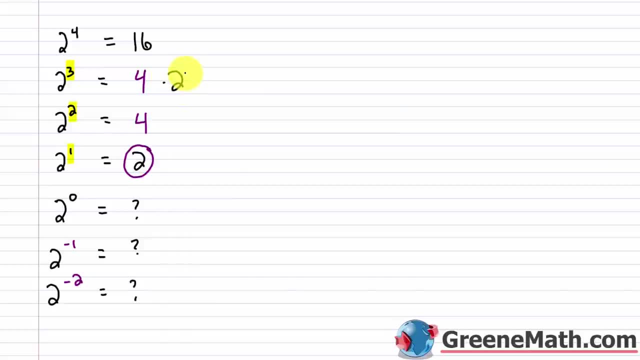 which is 4, and multiply it by another factor, another factor of 2.. That would give me 8.. Again, if I go up 1 in terms of my exponent, I go to 2, to the fourth power. If I don't know what that is, I can just take 8, which is the result from the 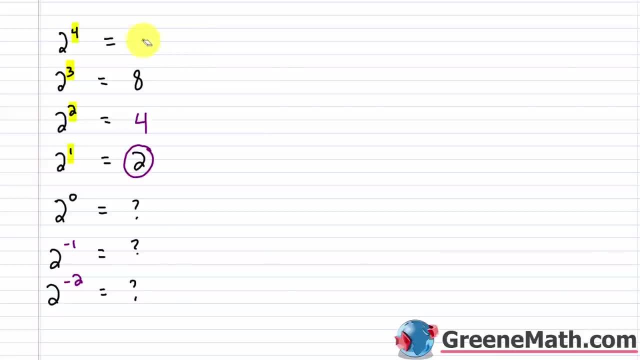 previous one and again multiply it by 2.. 8 times 2 is 16.. Now that's obvious, because each time I increase my exponent by 1, I'm basically taking the previous answer and I'm multiplying by another factor of 2.. What happens if I go down, though? Now I'm going to be dividing The opposite of 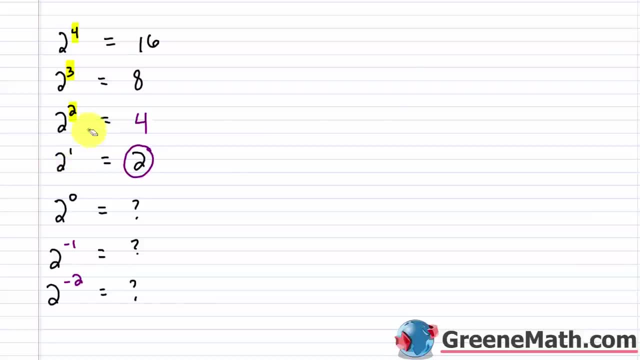 multiplication is division. In other words- let me erase this real quick- If I start out at 2 to the fourth power, the exponent is 4.. If I go down to 2 to the third power, I've decreased my exponent by 1.. If I didn't know what any of these were, I could just start with 16 and say: okay well. 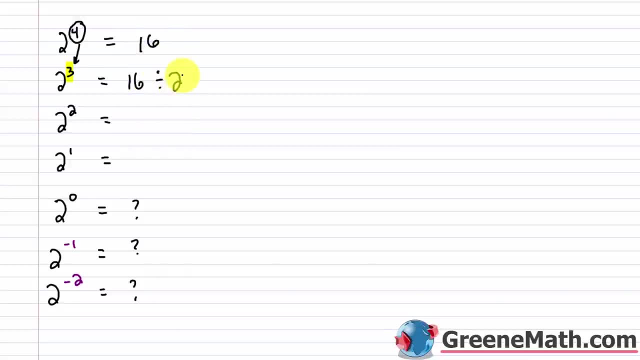 I have 16 here. I would just divide by 2.. I'm just going to end up with the number 8, because essentially what I'm doing is I'm saying: okay, I had 2 to the fourth power, which is 2 times 2 times 2 times 2.. Now I'm going to remove a factor of 2. 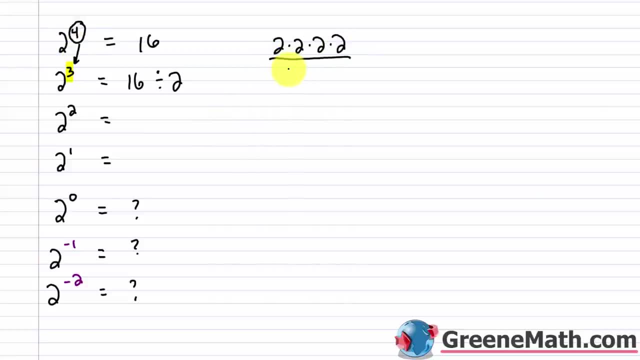 because I'm decreasing my exponent by 1.. Essentially, I'm dividing by 2 so that I can cancel one factor out. Now I have 2 cubed, which is this: right here I'm dividing that previous result, which was 16, by 2, and now I'm going to get to 8.. 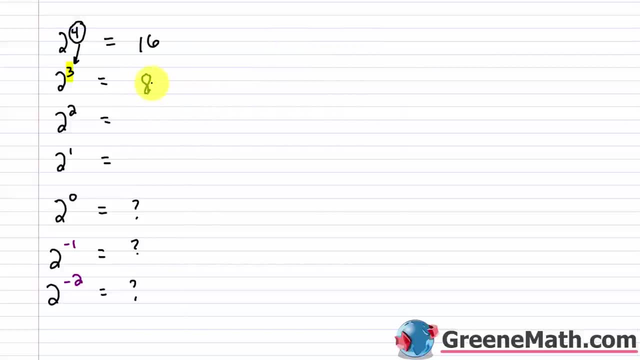 Now I'm going to get to 8.. I can keep doing this, going all the way down. In other words, if I want 2 squared, I take 8, I divide it by 2, and I get to 4.. If I want 2 to the first power. 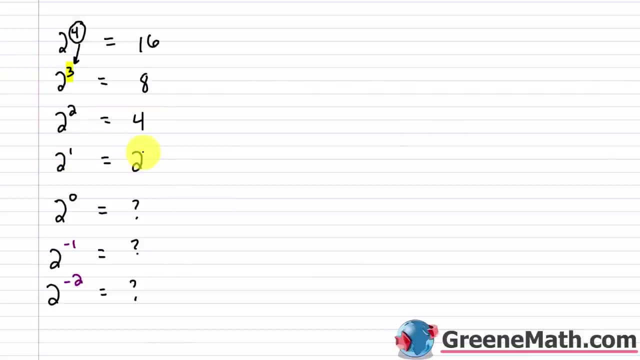 I take 4,, I divide it by 2, and I get 2.. If I want 2 to the power of 0, I take 2, and I divide it by 2, and I get 1.. I get 1.. This is 2 over 2, and this equals 1.. 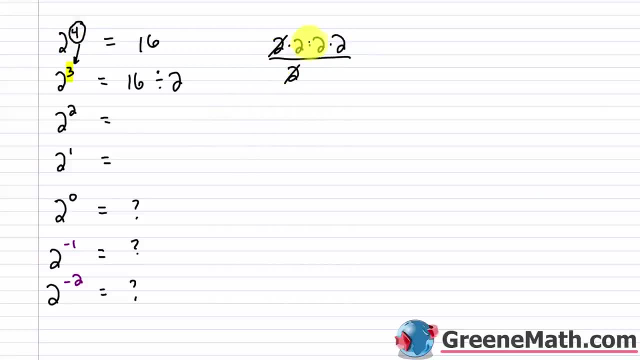 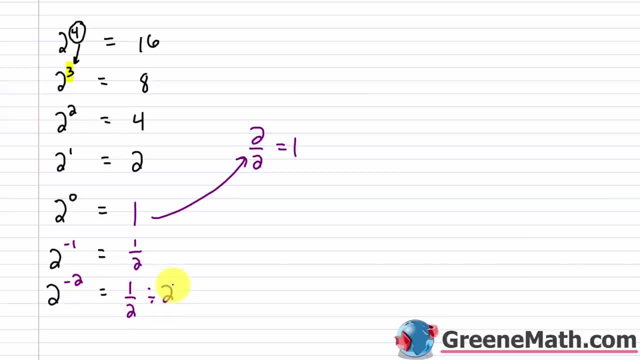 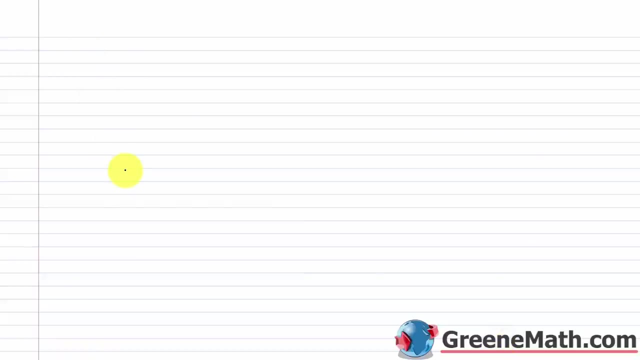 one half divided by 2 or you can think of it as one half divided by 2 over 1 and we know this equals one half times one half which equals one fourth. Let me show you another example real quick and then I'm going to give you a few rules that you want to write down. Let's start out with a base of 3 and do the same thing. If I have 3 cubed or you could say 3 to the third power 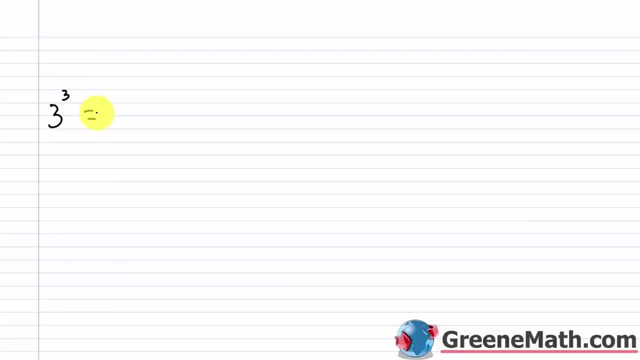 we know this is 3 factors of 3 or 27. 3 times 3 is 9. 9 times 3 is 27. 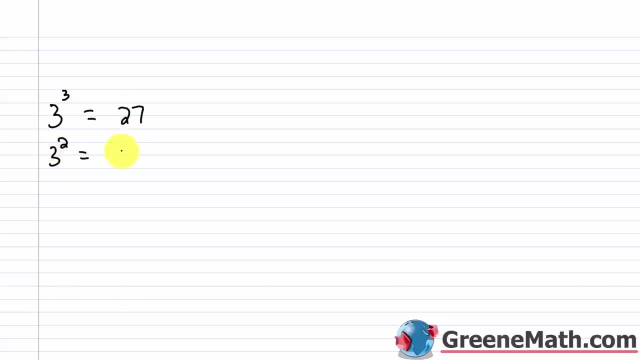 What about 3 squared? 3 times 3 is 9. What about 3 to the first power? We know that's 3. Then 3 to the power of 0. Let's do 3 to the power of negative 1 and 3 to the power of negative 2. 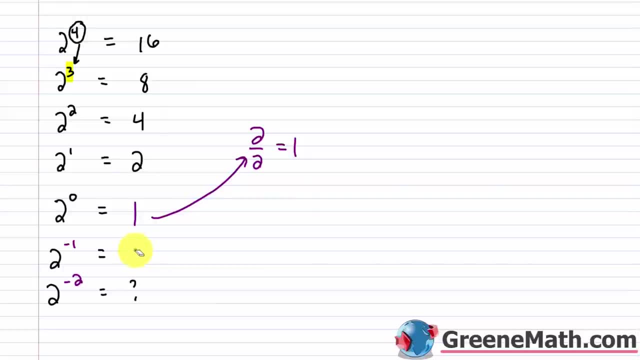 If I want 2 to the power of negative 1,, I take 1, and I divide it by 2.. So that's 1 over 2, or 1 half. If I want 2 to the power of negative 2,, I take 1 half and I divide it by 2.. So 1 half. 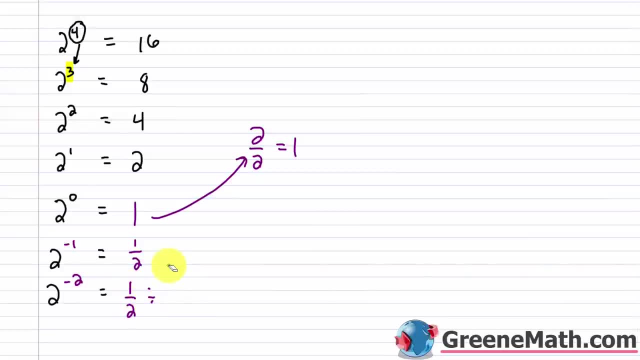 divided by 2, or you can think of it as 1 half divided by 2 over 1, and we know this equals 1 half times 1 half, which equals 1. fourth, Now I'm going to give you another example real quick, and then I'm going to give you a few rules. 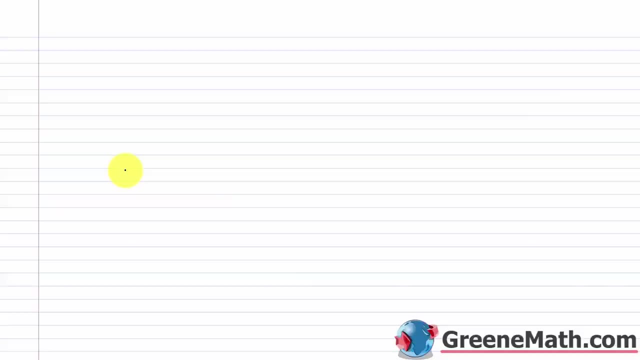 that you want to write down. Let's start out with a base of 3 and do the same thing. If I have 3 cubed, or you could say 3 to the third power, we know this is 3 factors of 3, or 27.. 3 times 3 is. 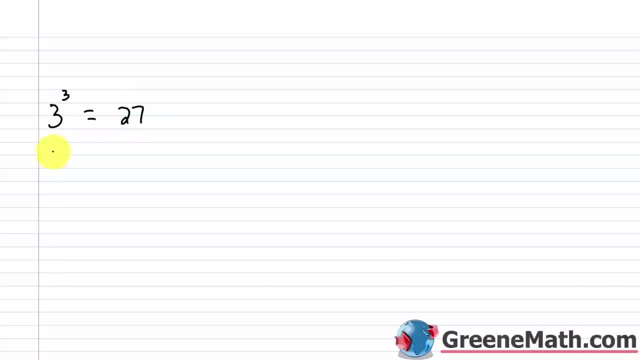 9.. 9 times 3 is 27.. What about 3 squared 3 times 3 is 9.. What about 3 to the first power? We know that's 3.. Then 3 to the power of 0.. 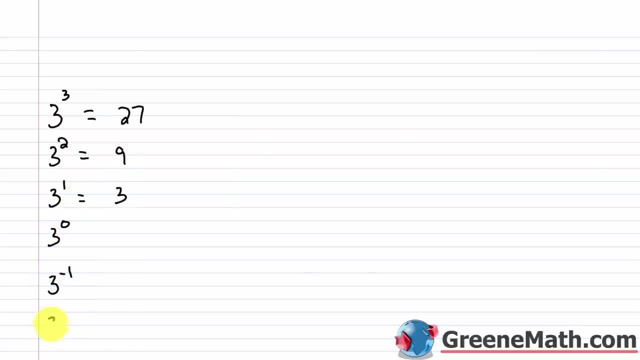 Let's do 3 to the power of negative 1, and 3 to the power of negative 2.. Again, as I go from here to here, as I decrease the exponent by 1,, I just divide this answer by the base. So in other words, 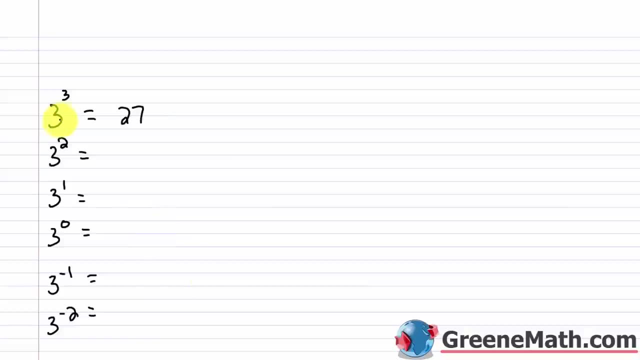 if I erase all this and I don't know any of it. if I want to go from a known result of 3 cubed, which is 27,, to an unknown result of 3 squared, all I do is take the result here and divide by 3.. 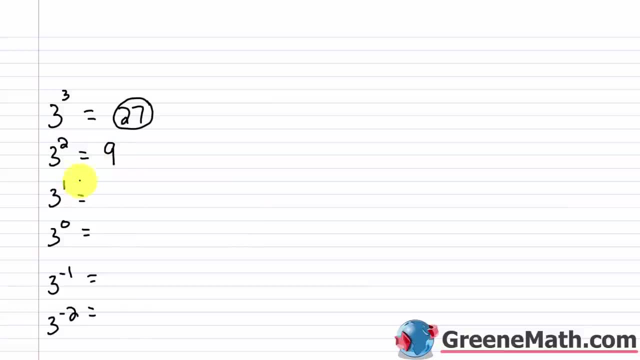 27 divided by 3 is 9.. To get to here, 9 divided by 3 is 3.. To get to here, 3 divided by 3 is 1.. Again, 3 to the power of 0 is 1.. To get to here, 3 to the power of negative 1.. Okay, 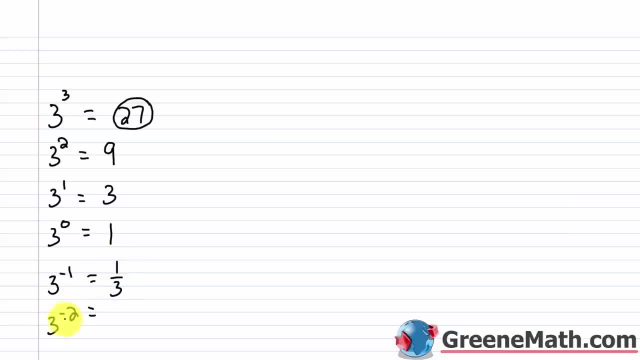 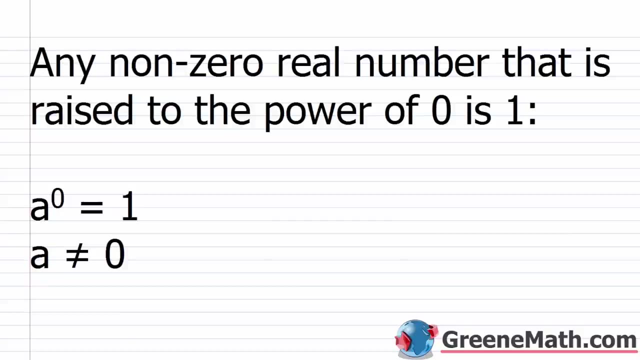 1 divided by 3 is 1 third. To get to here, 1 third divided by 3 is 1 ninth. So in each example we saw: 2 to the power of 0 was 1, and 3 to the power of 0 was 1.. 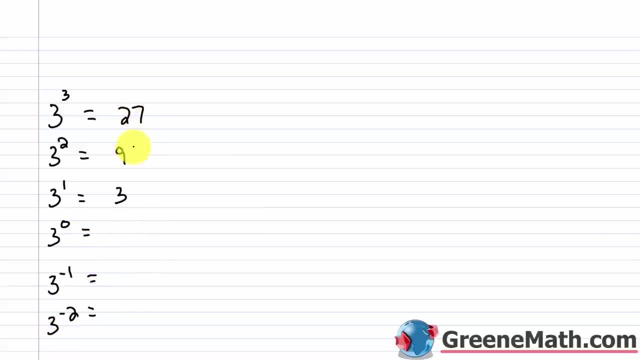 Again as I go from here to here as I decrease the exponent by 1 I just divide this answer by the base. So in other words if I erase all this and I don't know any of it if I want to go from a known result of 3 cubed which is 27 to an unknown result of 3 squared all I do is take the result here and divide by 3. 27 divided by 3 is 9. To get to here 9 divided by 3 is 3. To get to here 3 divided by 3 is 1. Again 3 to the power of 0 is 1. To get to here 3 divided by 3 is 1. Again 3 to the power of 0 is 1. To get to here 3 divided by 3 is 1. 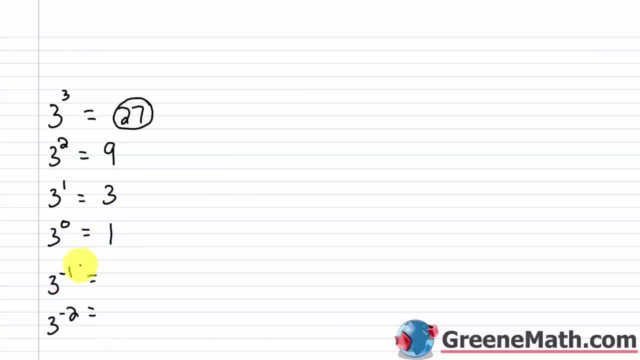 To get to here 3 to the power of negative 1. Okay 1 divided by 3 is 1 third. To get to here 1 third divided by 3 is 1 ninth. So in each example we saw 2 to the power of 0 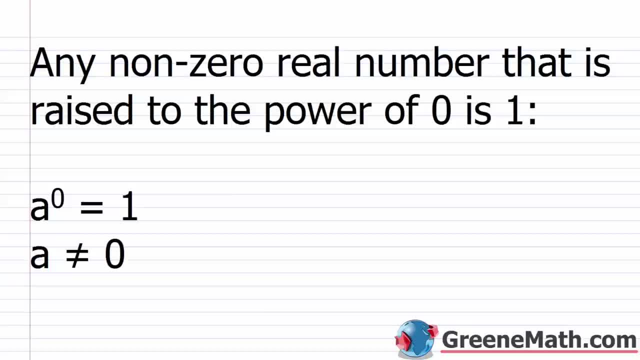 was 1 and 3 to the power of 0 was 1 also. So here's the rule that you want to write down and memorize. Any non-zero non-zero real number that is raised to the power of 0 is 1. 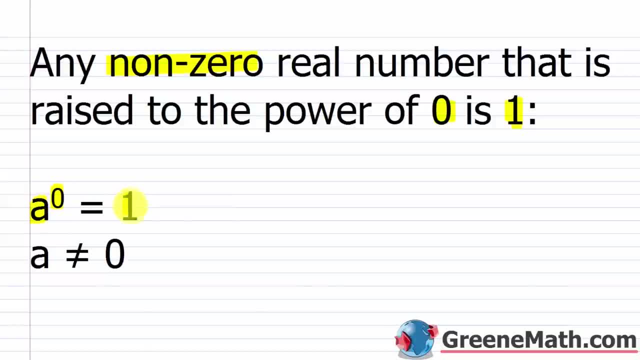 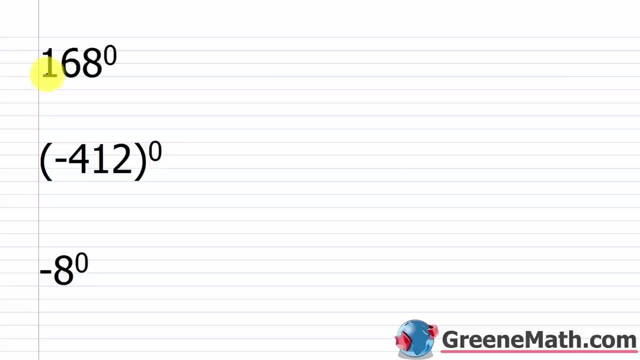 So a raised to the power of 0 is 1 and a is any real number but a is not allowed to be 0. Okay so a is not going to be 0. So any number you can pick doesn't matter what it is. Let's say I have 1032. If I raise it to the power of 0 it is equal to 1. Because essentially what a to the power of 0 is is it's a over a. It's the same number divided by itself and we know that a to the power of 0 is 1. Any non-zero number divided by itself is 1. So here are some very very easy examples and I'm sure you're going to see stuff like this in your textbook. So you have the number 168 raised to the power of 0. This is equal to 1. You have the amount negative 412 and this is inside of parentheses. So everything here is raised to the power of 0 and so this is equal to 1. And then you have the opposite of 8 raised to the power of 0. Again remember this rule. So this is equal to negative 1 times 8 to the power of 0. 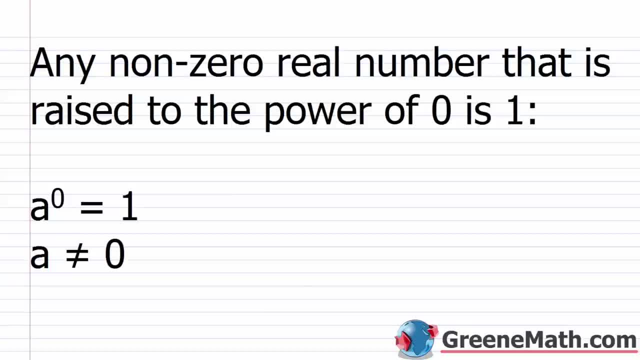 So here's the rule that you want to write down and memorize: Any non-zero, non-zero real number that is raised to the power of 0 is 1.. So a raised to the power of 0 is 1, and a is any real number. 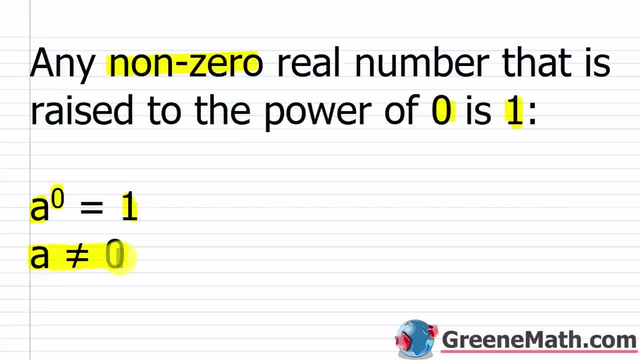 but a is not allowed to be 0. Okay, so a is not going to be 0. So any number you can pick, doesn't matter what it is. Let's say I have 1032.. If I raise it to the power of 0, it is equal to 1.. Because essentially, what a to the power of 0 is? 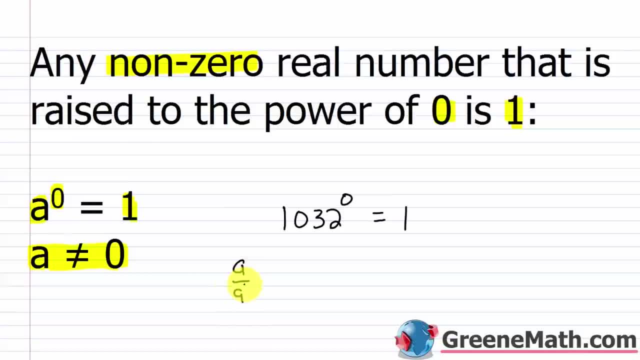 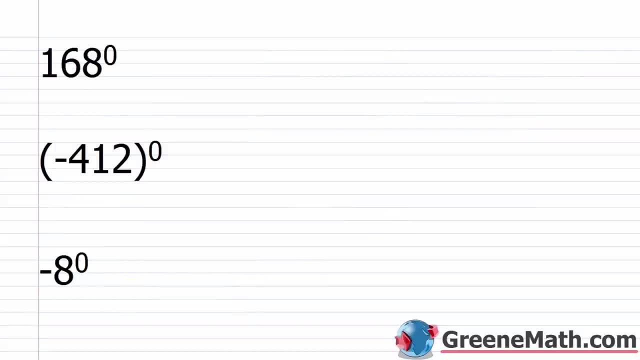 is: it's a over a. It's the same number divided by itself, and we know that any non-zero number divided by itself is 1.. So here are some very, very easy examples, and I'm sure you're going to see stuff like this in your textbook. So you have the number 168 raised to the power of 0.. 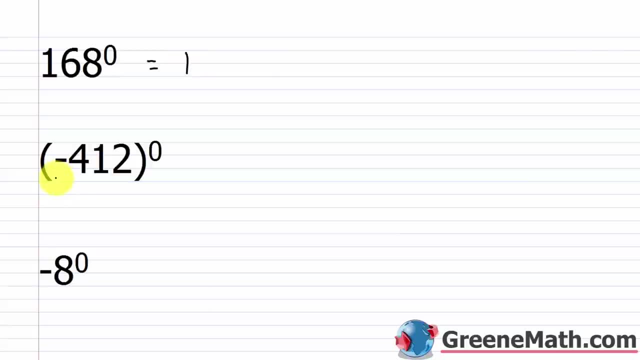 This is equal to 1.. You have the amount negative 412, and this is equal to 1.. So you have the amount negative 412, and this is equal to 1.. So you have the amount negative 412, and this is equal to 1.. So you have the amount negative 412,. 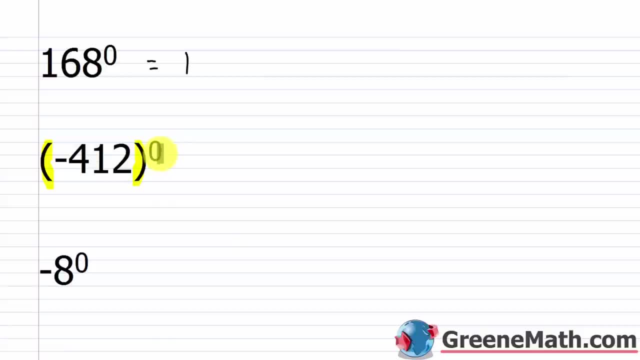 inside of parentheses. So everything here is raised to the power of 0,, and so this is equal to 1.. And then you have the opposite of 8 raised to the power of 0. Again, remember this rule. So this is equal to negative 1 times 8 to the power of 0.. 8 to the power of 0 is 1,. 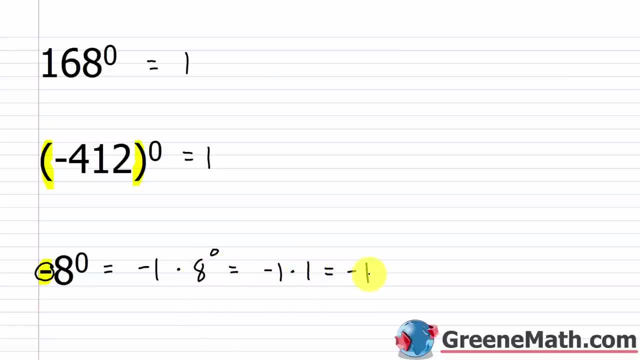 so this is negative 1 times 1, which equals negative 1.. Pay close attention to that, because for sure your teachers are going to try to trip you up with these, And then, of course, the same rules are going to apply when we work with variables. But again, you cannot raise. 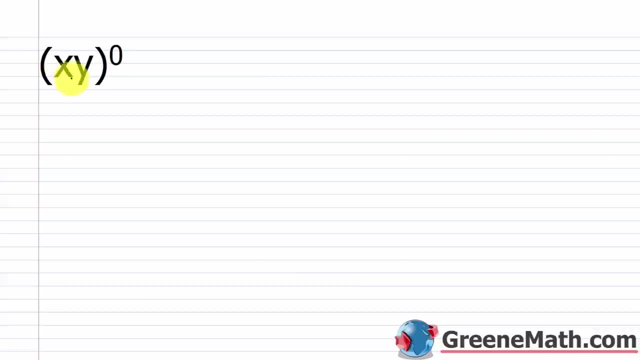 0 to the power of 0. So we have x, y. This is raised to the power of 0. It's inside of parentheses. So this is equal to x to the power of 0 times y to the power of 0, and each is going. 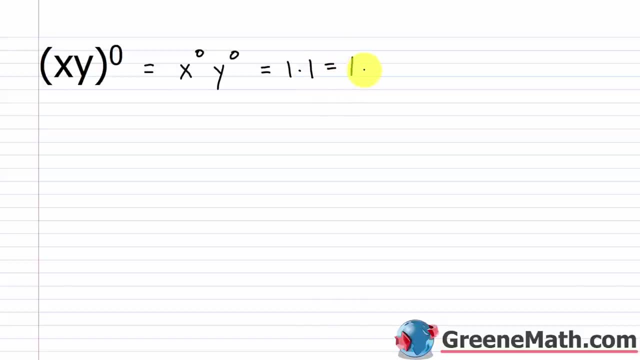 to be equal to 1.. So you get 1 times 1, or just 1.. But kind of the shortcut is to realize that, okay, both are raised to the power of 0. So this whole thing is raised to the power of 0. So that's. 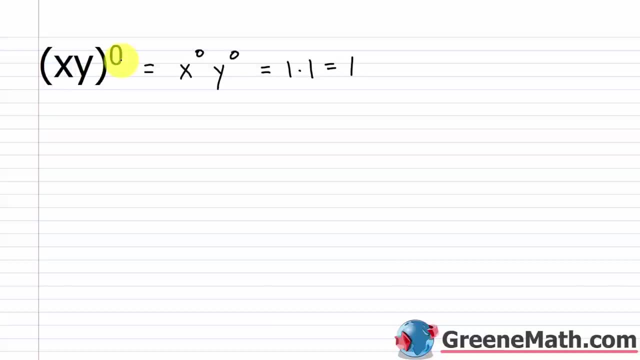 just going to be equal to 1.. And again, you're not going to see this at first, but recall that you can't divide by 0. And so x and y both have a limitation here. Neither one can be allowed to be. 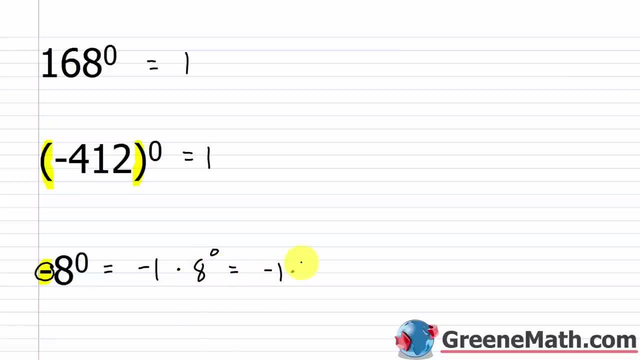 8 to the power of 0 is 1. So this is negative 1 times 1 which equals negative 1. Pay close attention to that because for sure your teachers are going to try to trip you up with these. And then of course the same rules are going to apply when we work with variables but again you cannot raise 0 to the power of 0. So we have xy. this is raised to the power of zero. It's inside of parentheses. So this is equal to x to the power of zero times y to the power of zero, and each is gonna be equal to one. 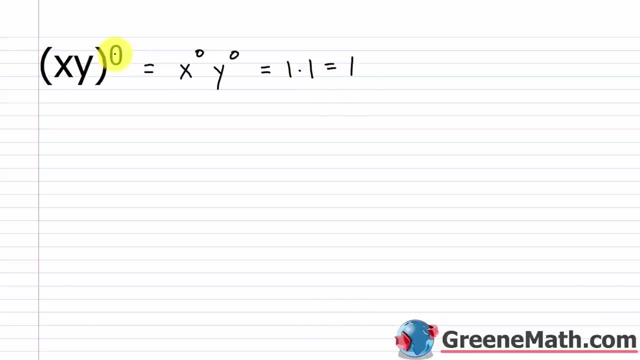 So you get one times one or just one. But kind of the shortcut is to realize that, okay, both are raised to the power of zero, so this whole thing is raised to the power of zero, so that's just gonna be equal to one. 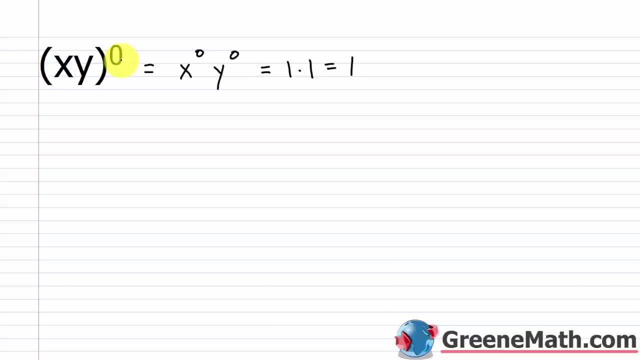 And again, you're not gonna see this at first, but recall that you can't divide by zero, and so x and y both have a limitation here. Neither one can be allowed to be equal to zero. 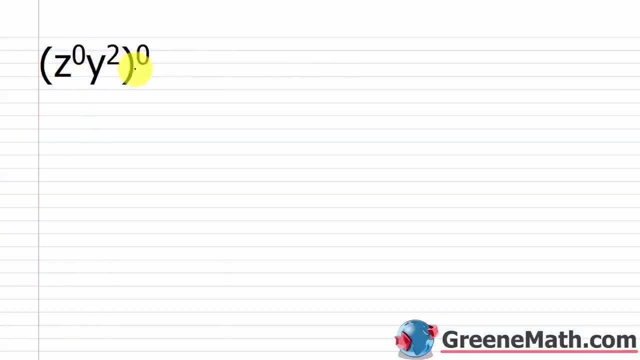 But what about something like z to the power of zero y squared, and then this is all raised to the power of zero? 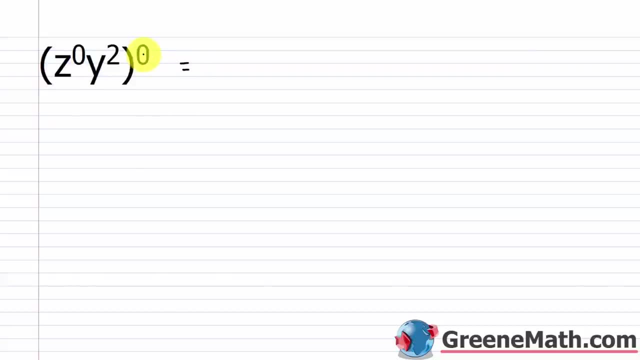 Well, you don't need to go through anything. You could do it individually if you wanted to. You could do power to power rule and go, okay, well, z to the power of zero times zero, and then this is multiplied by y to the power of two times zero. In the end, anything times zero is just zero. So you can kind of figure out what's going to happen if you kind of skip this step, 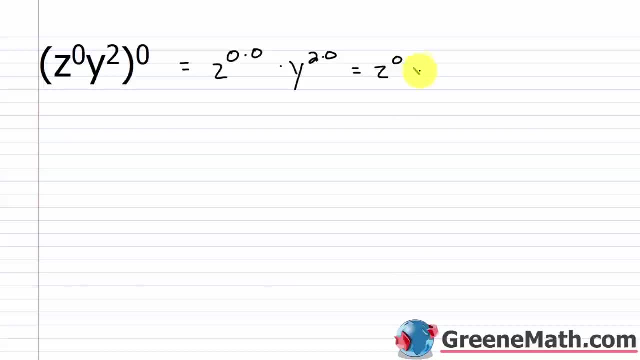 because it ends up being z to the power of zero times y to the power of zero, which is equals one times one, or one. But again, the shortcut is to realize that everything here inside the parentheses is raised to the power of zero, so the result is just gonna be one. 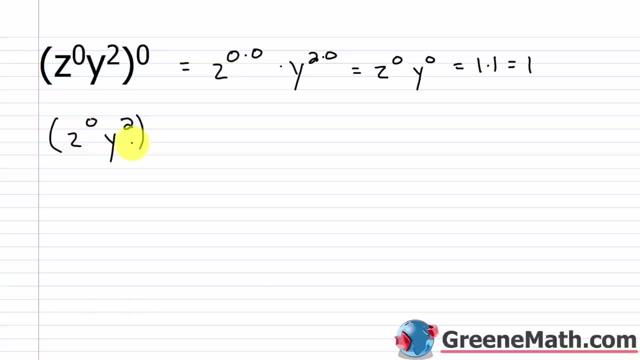 So I could have just as easily said, okay, z to the power of zero, y squared, everything's raised to the power of zero, so this just equals one. 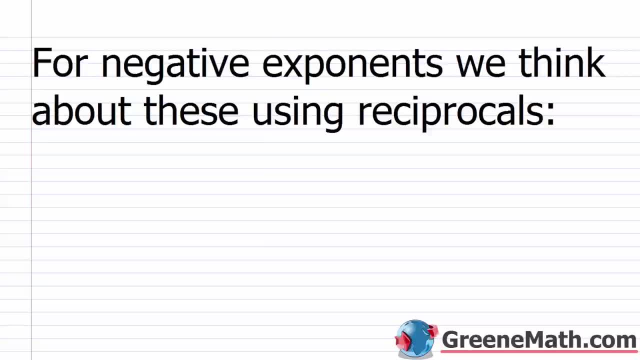 All right, so for raising something to the power of zero, very, very simple. Remember, you raise any non-zero number to the power of zero, it's just one. 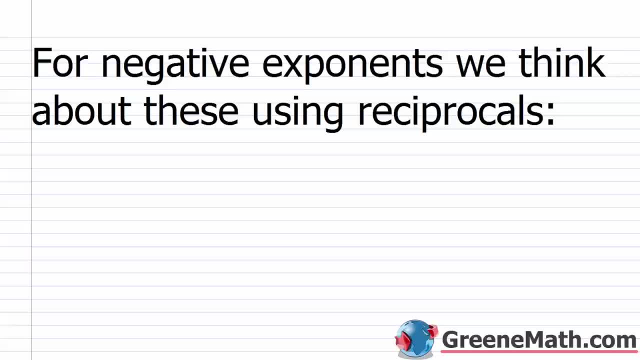 Okay, just memorize that. You're gonna use that a lot moving forward. 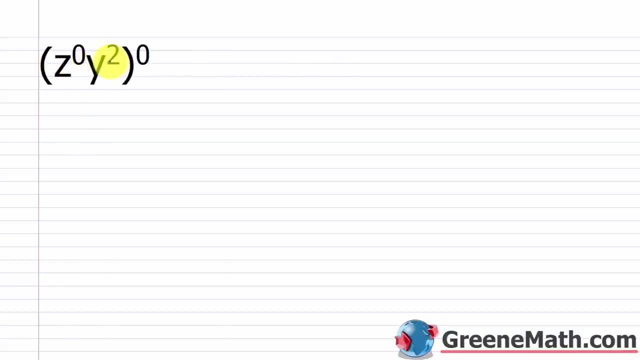 equal to 0.. But what about something like z to the power of 0, y squared, and then this is all raised to the power of 0?? Well, you don't need to go through anything. You could do it individual if you wanted to. You could do power to power rule and go. okay. well, z to the power of 0 times 0,. 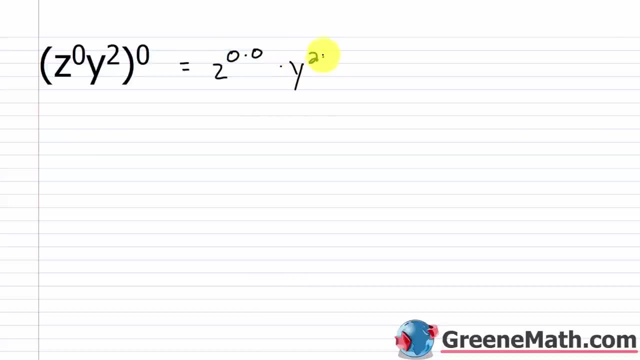 then this is multiplied by y to the power of 2 times 0. In the end, anything times 0 is just 0. So you can kind of skip this step, because it ends up being z to the power of 0 times y to the power of. 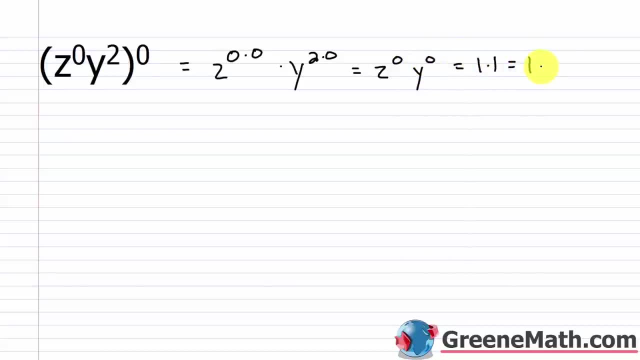 0,, which is equals 1 times 1, or 1.. But again, the shortcut is to realize that everything here inside the parentheses is raised to the power of 0. So the result is just going to be 1.. So I could. 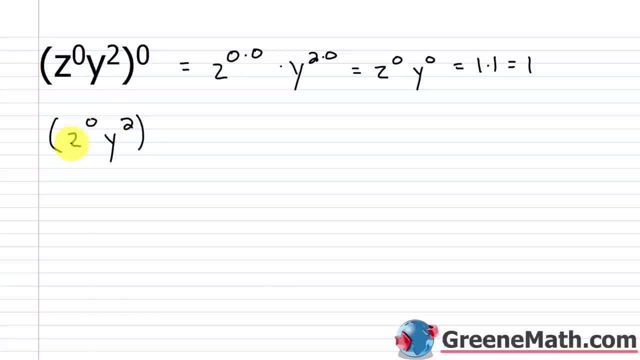 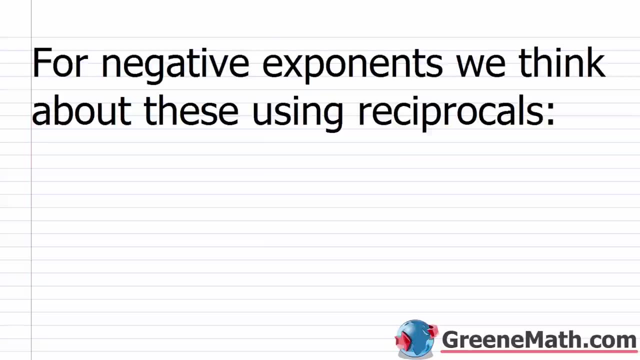 have just as easily said: okay, z to the power of 0, y squared, everything's raised to the power of 1.. All right, so for raising something to the power of 0,, very, very simple. Remember: you raise any non-zero number to the power of 0,, it's just 1.. Okay, just memorize that, You're. 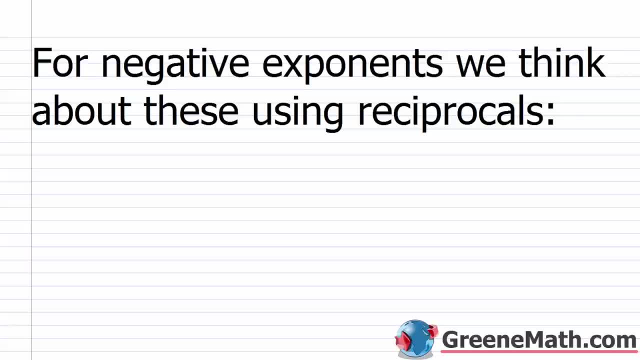 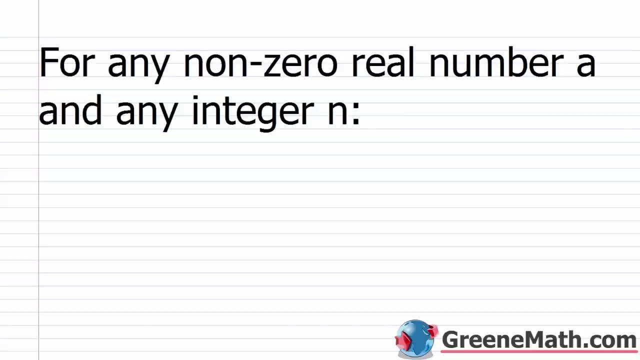 going to use that a lot moving forward. So now let's talk about negative exponents. So for negative exponents, we think about these using reciprocals. So I want you to recall that we had 2 to the power of negative 1, and this was equal to 1 over 2.. 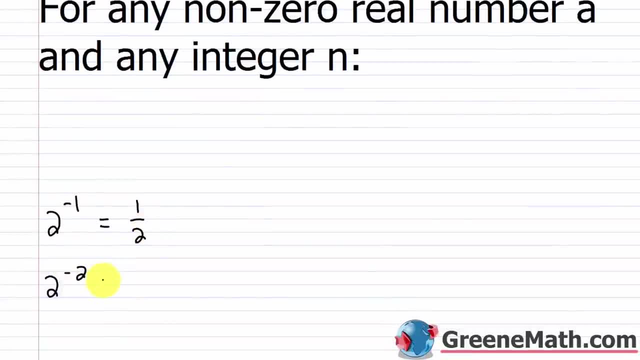 Or 1 half. We had 2 to the power of negative 2, and this was equal to 1. fourth, We saw 3 to the power of negative 1, this was equal to 1. third, We saw 3 to the power of negative 2, this was equal. 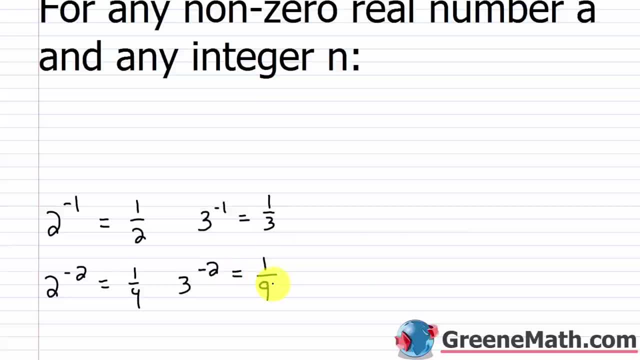 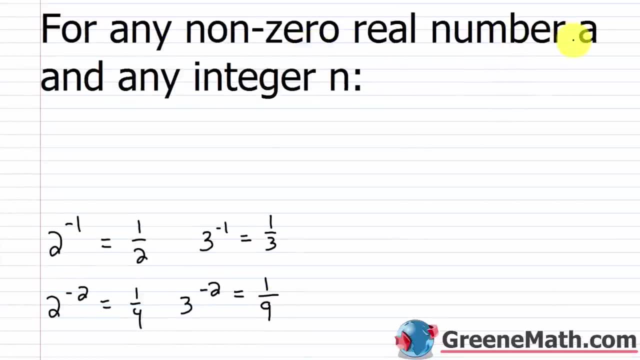 to 1 over 3 squared or 1 ninth. Now I'm going to give you the rule here: For any non-zero real number, a. okay, a just stands for any non-zero real number and any integer n. 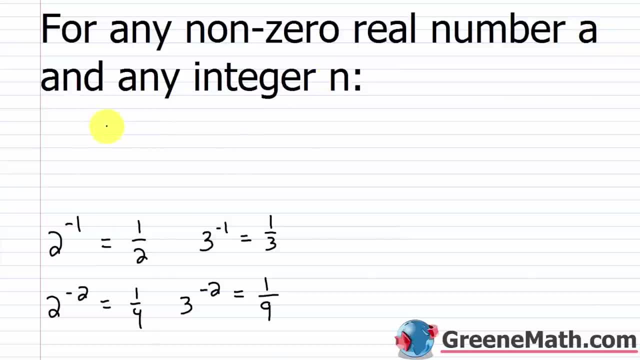 we have the following rule: So a raised to the power of negative n is going to be equal to 1 over a to the power of n. So you can just kind of substitute into this formula here and you'll never get the wrong answer. So in other words, a here in this specific example, is going to: 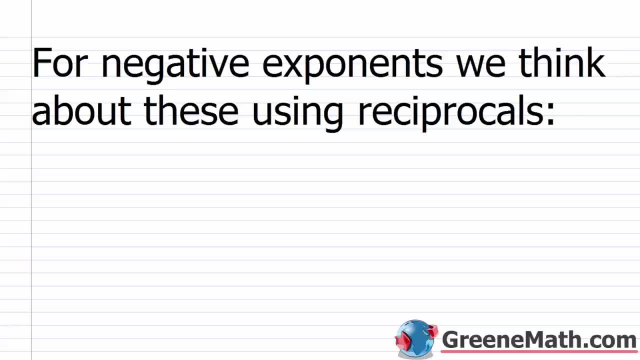 So now let's talk about negative exponents. So for negative exponents, we think about these using reciprocals. 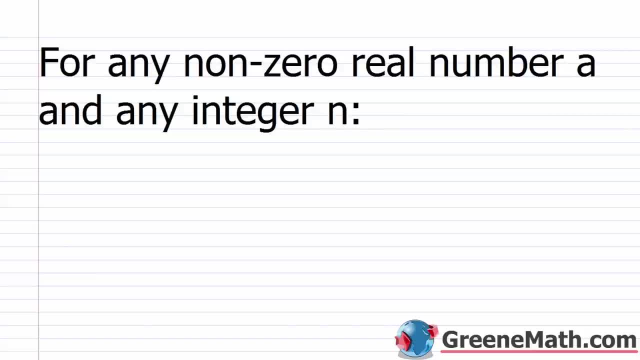 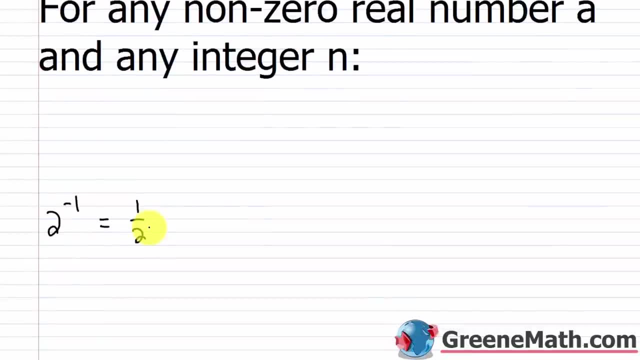 So I want you to recall that we had two to the power of negative one, and this was equal to one over two, or 1 1⁄2. We had two to the power of negative two, and this was equal to 1 4th. 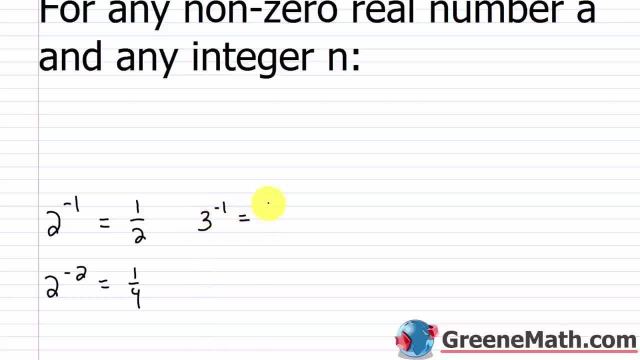 We saw three to the power of negative one. This was equal to 1 3rd. 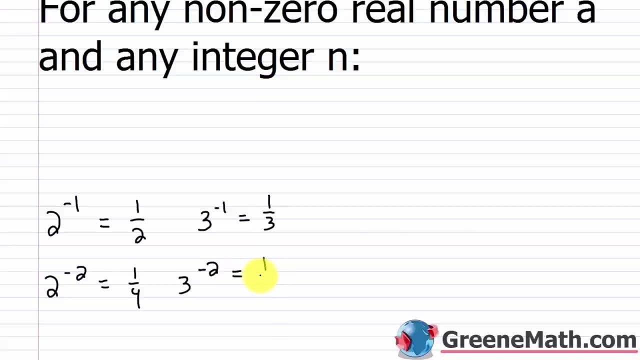 We saw three to the power of negative two. This was equal to one over three squared, or 1 9th. 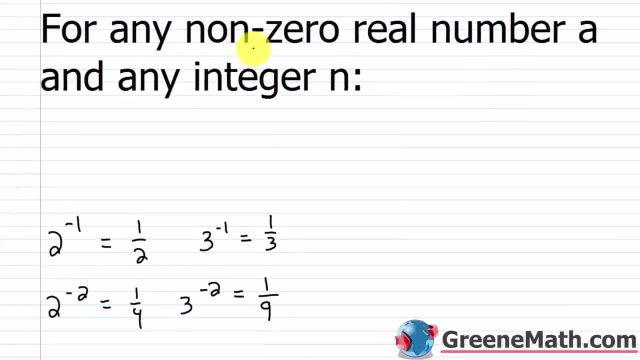 Now, I'm gonna give you the rule here. For any non-zero real number, a, okay, a just stands for any non-zero real number, and any integer n, we have the following rule. So a raised to the power of negative one, raised to the power of negative n, is going to be equal to one over a to the power of n. 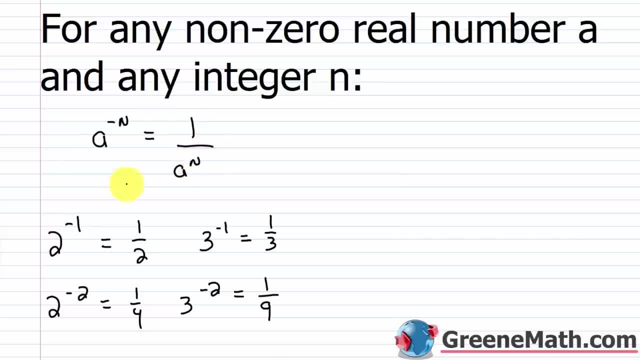 So you can just kind of substitute into this formula here, and you'll never get the wrong answer. 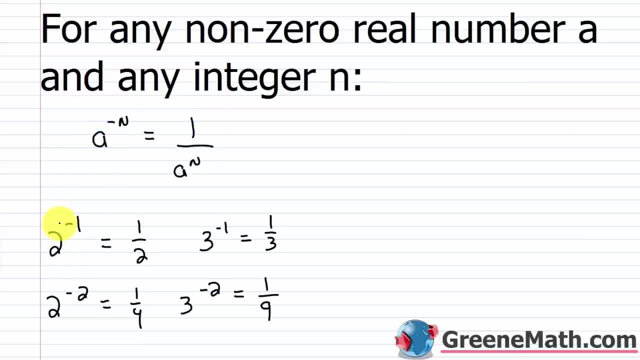 So in other words, a here, in this specific example, is going to represent two, right there. 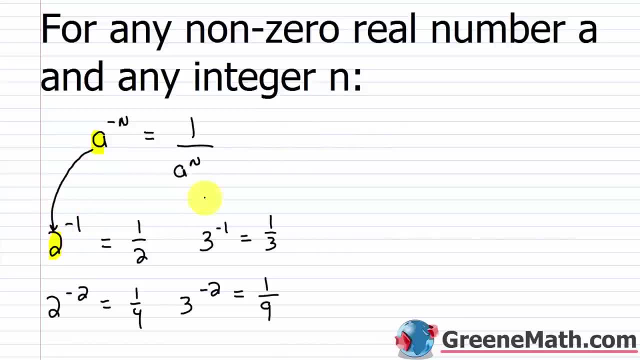 So then, all I would do is plug a two in where that is. So kind of to do this over here, I would have one, over, plug a two in for a, and then here I see that I have negative n, and then here I have positive n. 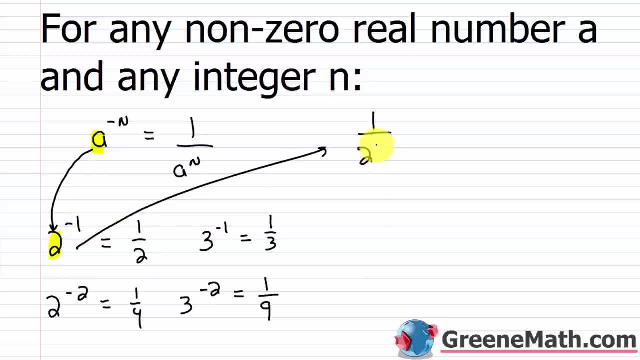 So in other words, this starts out as negative one, it becomes positive one, and two to the power of positive one is just two. 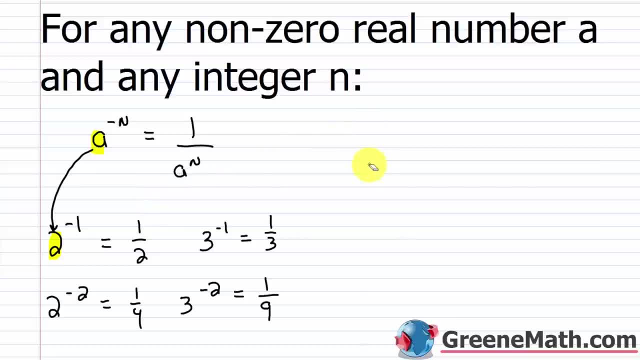 What we're doing here is we're taking the reciprocal of the base. So let's say I had something like 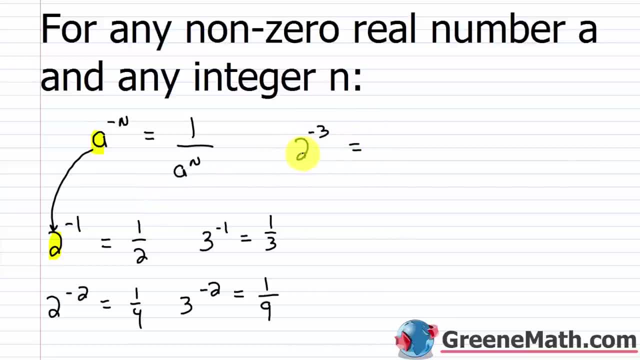 two to the power of negative three. I take the reciprocal of that guy, two, and that's gonna be one over two, or 1 1⁄2. 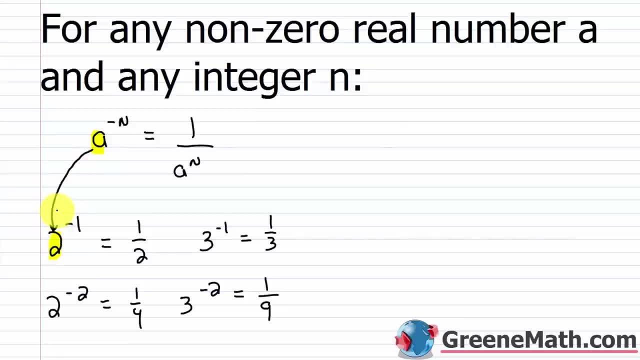 represent 2, right there. So then all I'm going to do is I'm going to do a little bit of a multiplication. So what I would do is plug a 2 in where that is So kind of to do this over here. 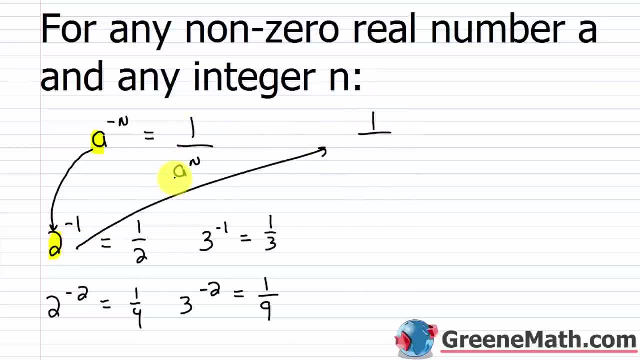 I would have 1 over, plug a, 2 in for a, and then here I see that I have negative n, and then here I have positive n. So in other words, this starts out as negative 1,, it becomes positive 1, and 2 to. 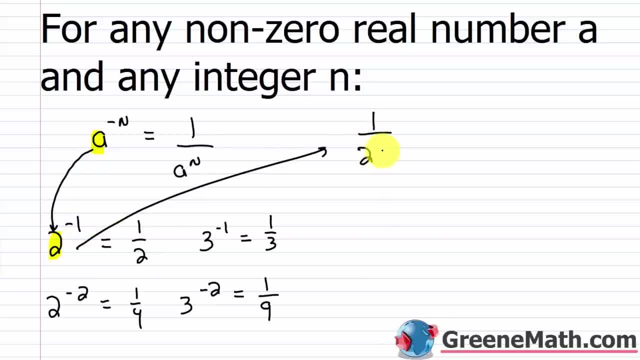 the power of positive 1 is just 2.. What we're doing here is we're taking the reciprocal of the base- So let's say I had something like 2- to the power of negative 3. I take the reciprocal of that guy, 2, and that's going to be 1 over 2, or 1 half, And then I'm raising 2 to the same exponent. 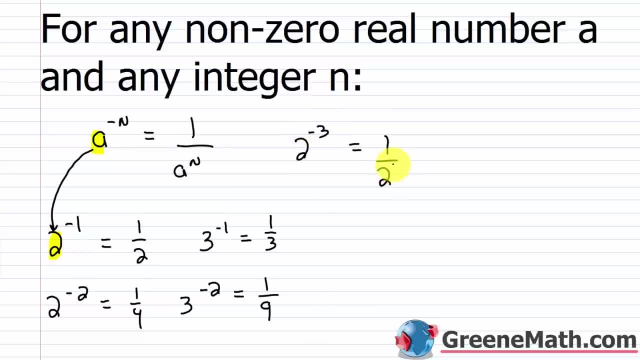 The only difference is, instead of it being negative, we make it positive. So 2 to the power of negative 3 is equal to 1 over 2 cubed, Or 2 to the power of negative 4 is equal to 1. 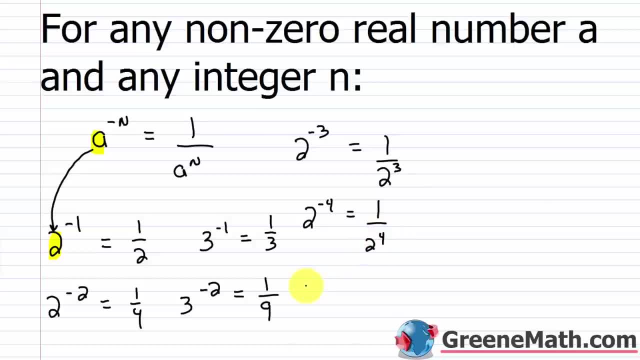 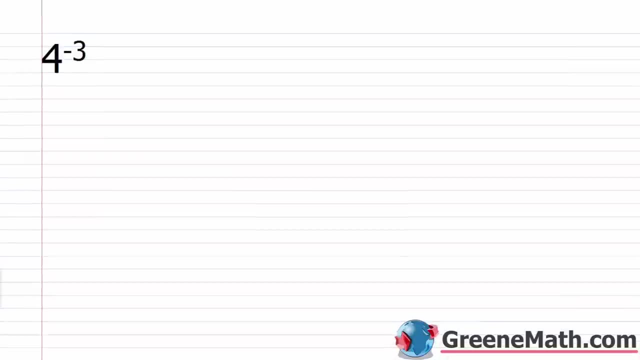 over 2 to the fourth, Or 2 to the power of negative 12 is equal to 1 over 2 to the power of 12.. It's not very complicated once you kind of memorize and do enough practice. Very, very straightforward rule, All right. so 4 to the power of negative 3.. What do we do here? 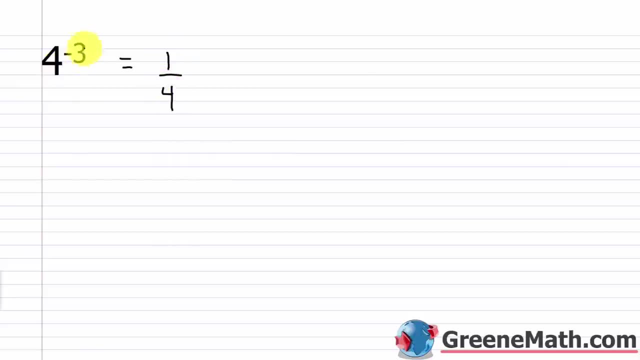 Flip the base so this becomes 1, fourth, and then this exponent is now going to be positive. It's still on 4, but it's just now just going to be positive. So 4 to the power of negative, 3 is. 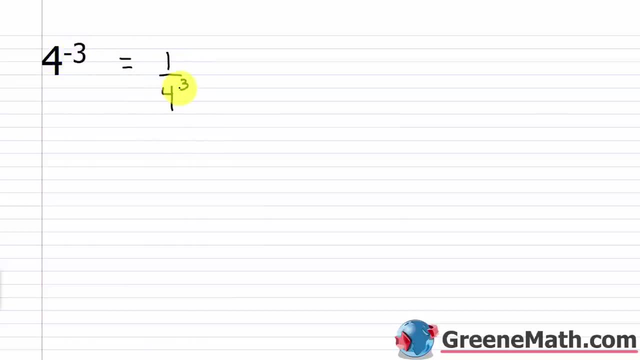 equal to 1 over 4 to the power of 3, or 1 over 4 cubed 6 to the power of negative 2.. Again, flip the base, So 6 will now be 1. sixth, and then make that exponent positive, So this is going to be 2.. 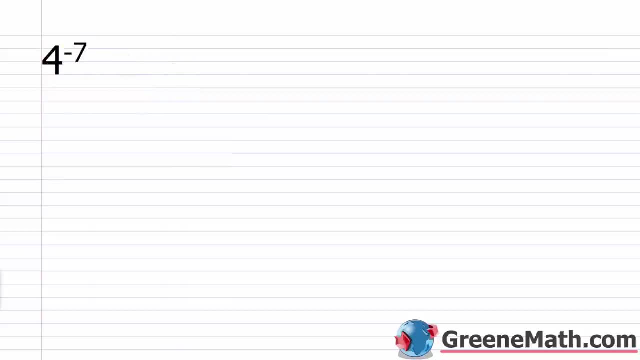 So 1 over 6, squared 4 to the power of negative 7.. So again, flip that base 4.. So this is going to be 1 over 4.. And then your exponent here, instead of being negative 7, is positive 7.. 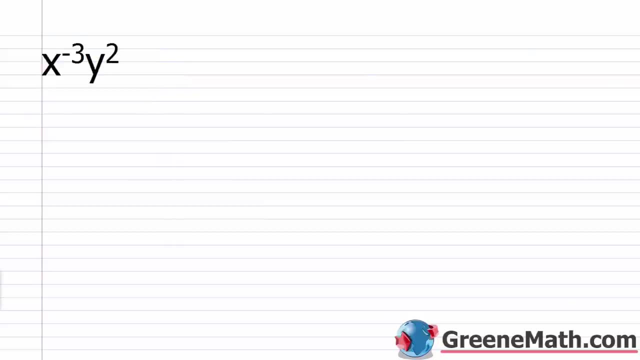 So this is 1 over 4 to the seventh power. What about x to the power of negative 3 y squared? Well, you can kind of separate these. Think about this as x to the power of negative 3 times y squared. So you can kind of separate these. Think about this as x to the power of. 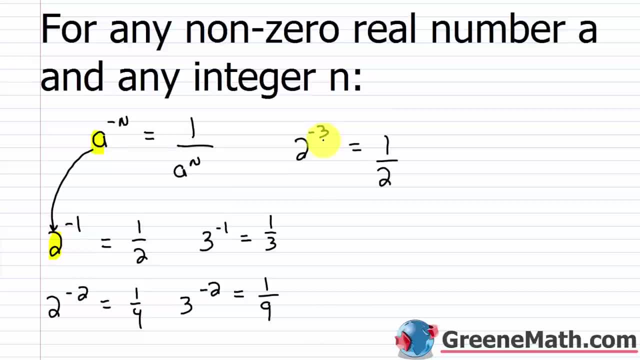 And then I'm raising two to the same exponent. The only difference is instead of it being negative, we make it positive. So two to the power of negative three is equal to one over two cubed. Or two to the power of negative four is equal to one over two to the fourth. Or two to the power of negative 12 is equal to one over two to the power of 12. 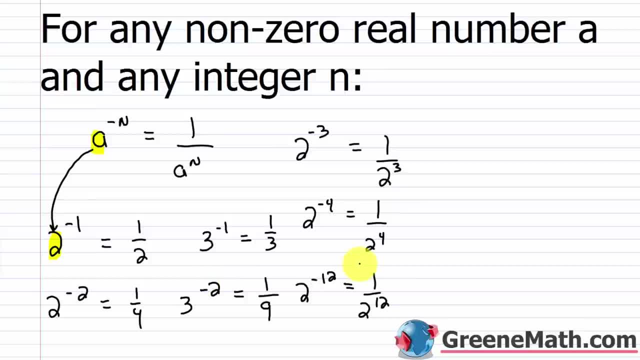 It's not very complicated once you kind of memorize, and do enough practice. 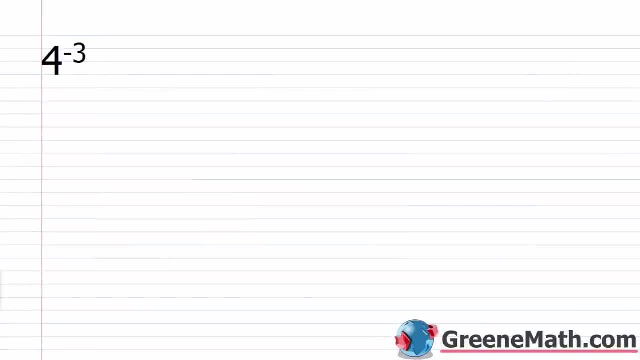 Very, very straightforward rule. All right, so four to the power of negative three. What do we do here? Flip the base, so this becomes 1⁄4, and then this exponent's now gonna be positive. 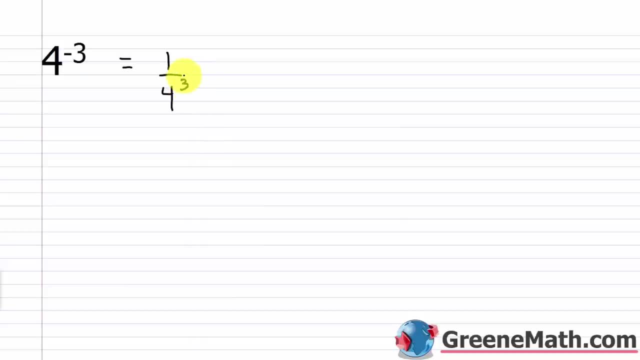 It's still on four, but it's just now just gonna be positive. 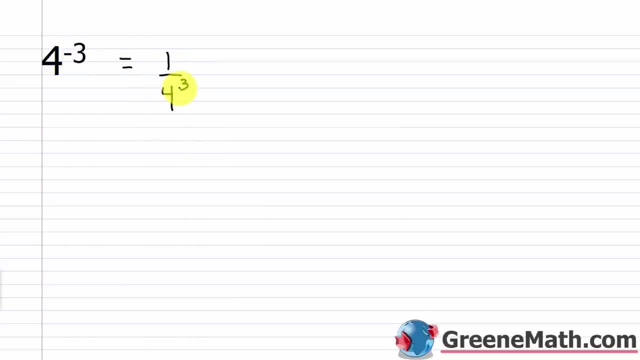 So four to the power of negative three is equal to one over four to the power of three, or one over four cubed. Six to the power of negative two. Again, flip the base. 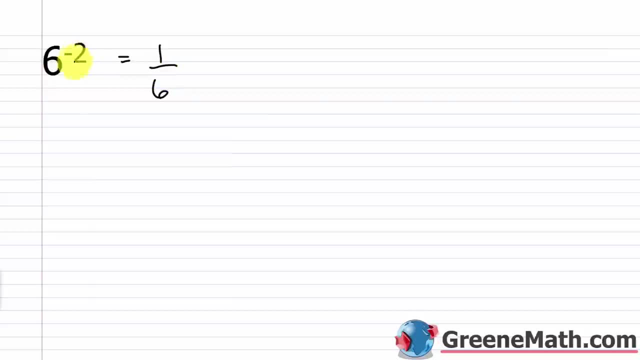 So six will now be 1⁶, and then make that exponent positive. So this is gonna be two. So one over six squared. 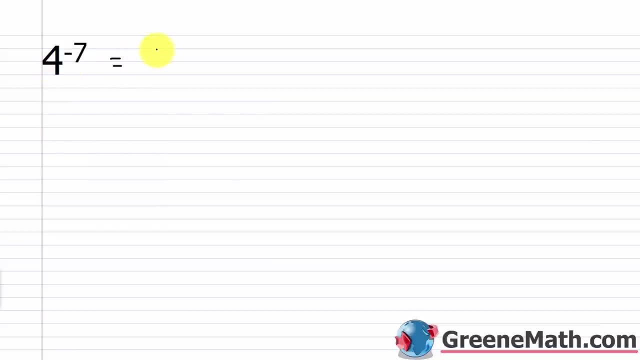 Four to the power of negative seven. So again, flip that base four. So this is gonna be one over four. And then your exponent here, instead of being negative seven, is positive seven. 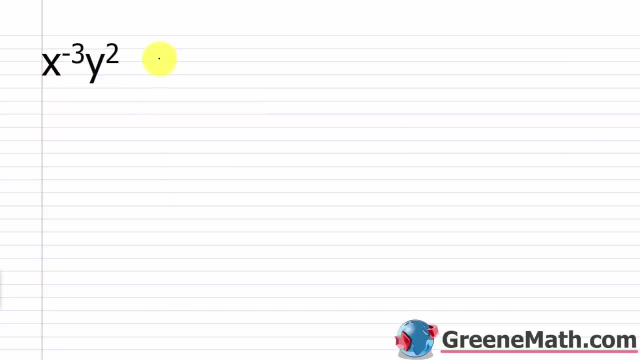 What about x to the power of negative three y squared? Well, you can kind of separate these. Think about this as x to the power of negative three times y squared like that. 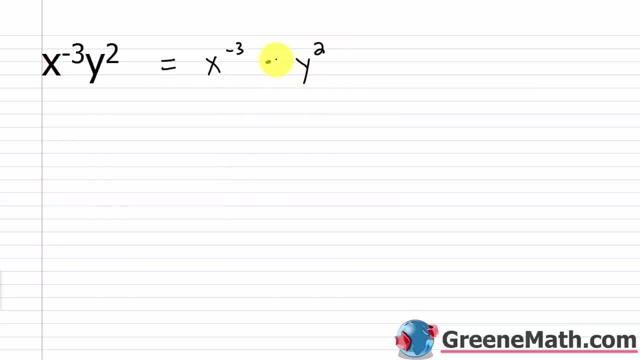 When you separate stuff with a multiplication sign, although you don't need it to imply multiplication, it kinda makes it easier for you to kind of separate these two in your mind. 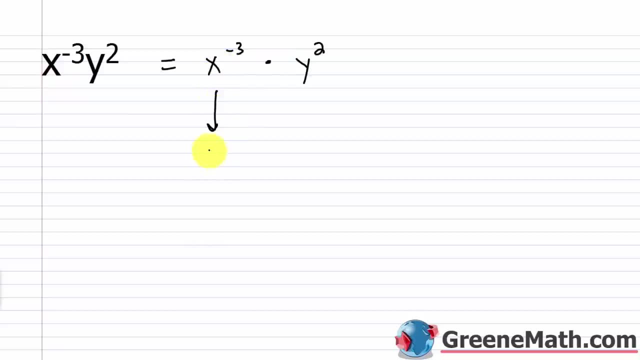 So this one right here is really one over x cubed, right? 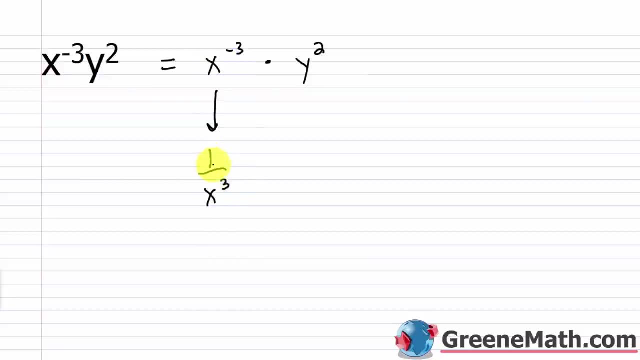 I have the base here, which is x. I take the reciprocal of that, so I get one over x. And then x is still gonna be raised to a power. I just make that power positive. 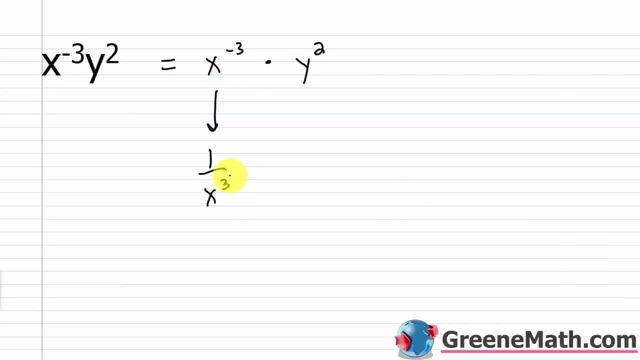 So instead of being raised to negative three, it's positive three. So really what this becomes is one over x cubed 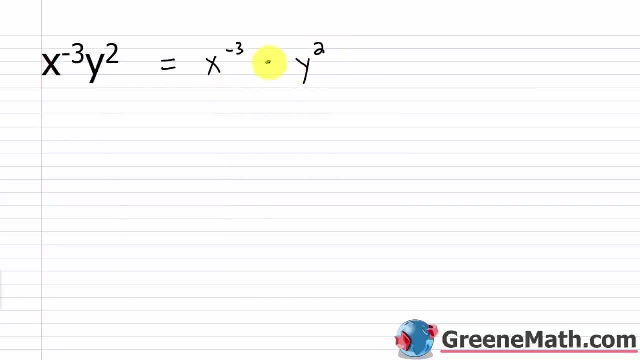 negative 3 y squared. Like that. When you separate stuff with a multiplication sign, although you don't need it to imply multiplication, it kind of makes it easier for you to kind of separate these two in your mind. So this one right here is really 1 over x cubed, right I have. 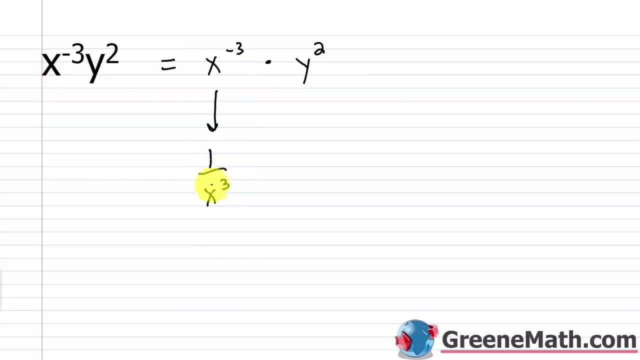 the base here, which is x. I take the reciprocal of that, so I get 1 over x, And then x is still going to be raised to a power. I just make that power positive. So instead of being raised to negative 3, it's positive 3.. So I'm going to make that power positive. So instead of being raised to 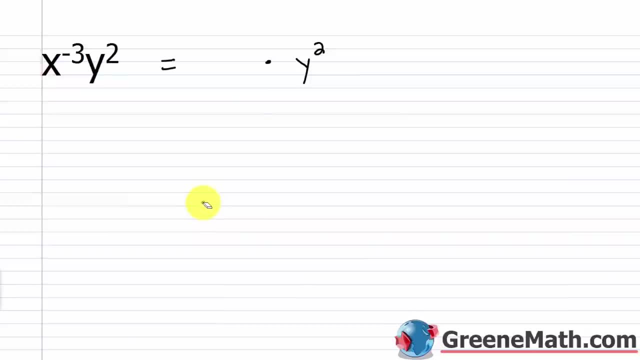 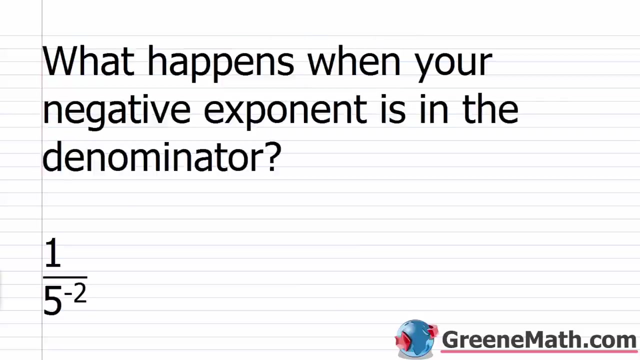 3.. So really, what this becomes is 1 over x cubed times y squared, which I can write as y squared over x cubed, right, Because y squared times 1 would just be y squared. So the next situation you're going to encounter is a negative exponent in the denominator. So what happens when your 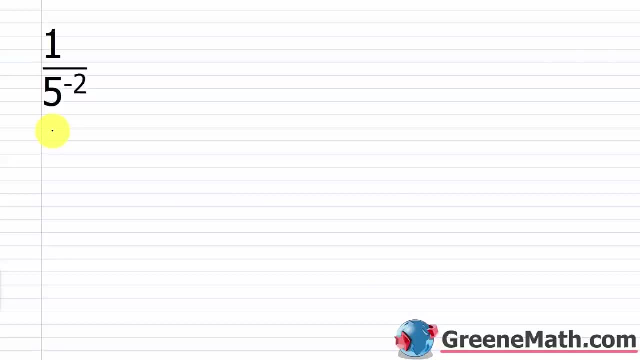 negative exponent is in the denominator. Well, all you really need to do is bring your denominator into the numerator And make the exponent positive. So I'm just going to take this guy up here and the exponent's going to be positive. So 5 comes up here. The exponent negative 2 becomes positive 2.. And this is times. 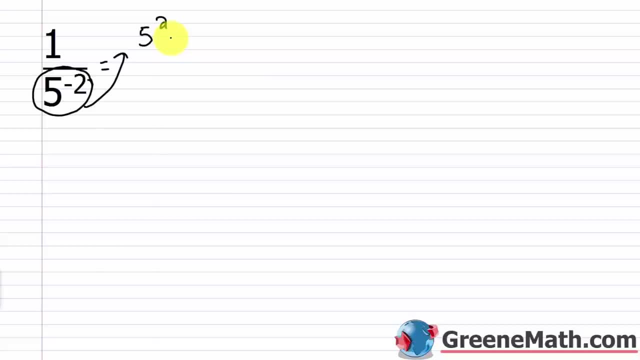 1, which is still going to be 5 squared. So 1 over 5 to the power of negative 2 is just equal to 5 squared, And if you want to think about this using the rule that I just gave you, let's suppose we. 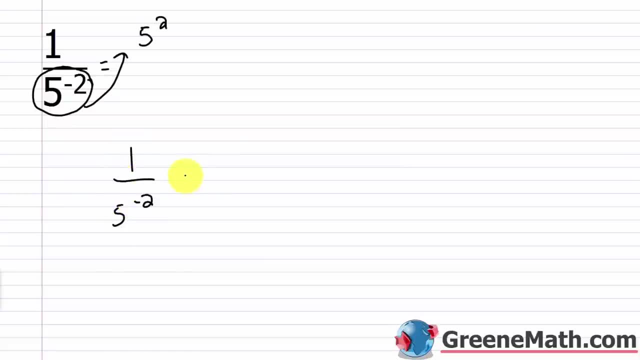 wrote this out: 1 over 5 to the power of negative 2.. So let's say this is equal to 1 over 1 divided by 5 to the power of negative 2, is 1 over 5 to the power of 2, or 5 squared right because this guy, we take the reciprocal, So that's. 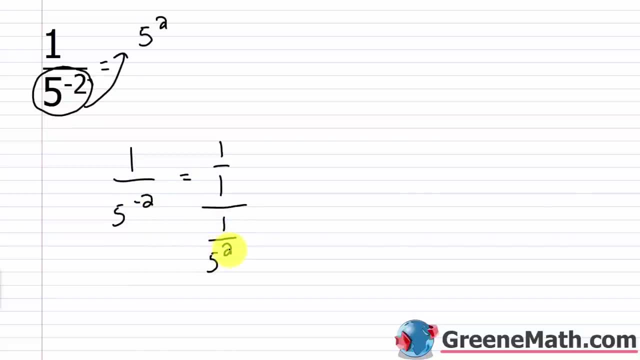 1 over 5. Make this guy positive. So raised to the power of 2.. Now I wrote this original 1 here as 1 over 1, so we could divide with fractions. So how do I divide fractions Again? 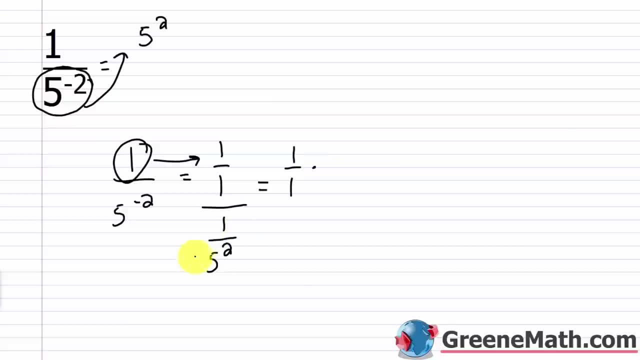 this part would stay the same. So I'll have 1 over 1 times the reciprocal of this guy, which would be five squared over one. At the end of the day, it's one times five squared, or five squared over one, which is just five squared. 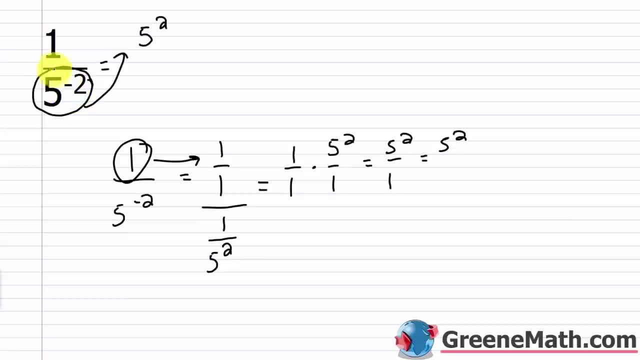 So again, the shortcut to that process is you're gonna take the number from the denominator that's raised to a negative power, bring it into the numerator, and then you're gonna take that exponent that's negative and you're gonna make it positive. 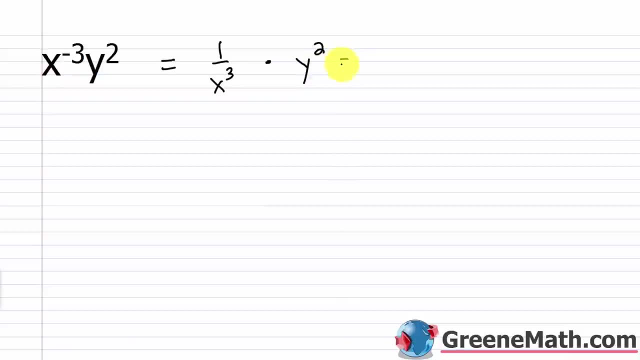 times y squared, which I can write as y squared over x cubed, because y squared times one would just be y squared. 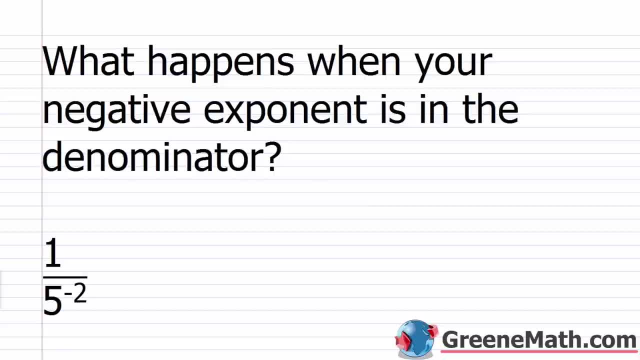 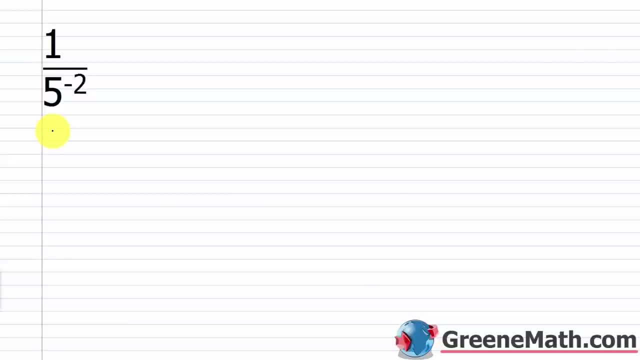 So the next situation you're gonna encounter is a negative exponent in the denominator. So what happens when your negative exponent is in the denominator? Well, all you really need to do is bring your denominator into the numerator and make the exponent positive. 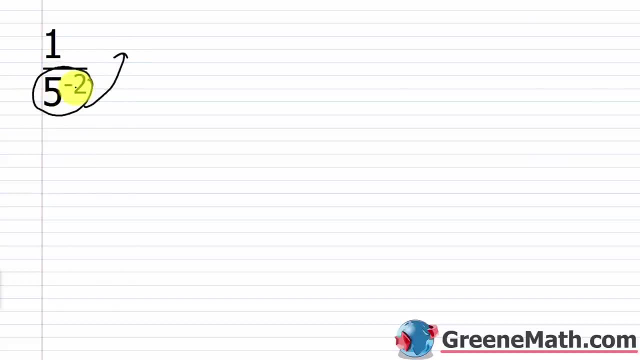 So I'm just gonna take this guy up here. this guy up here, and the exponent's going to be positive. So 5 comes up here, the exponent negative 2 becomes positive 2, and this is times 1, which is still going to be 5 squared. So 1 over 5 to the power of negative 2 is just equal to 5 squared. And if you want to think about this using the rule that I just gave you, let's suppose we wrote this out, 1 over 5 to the power of negative 2. So let's say this is equal to 1 over 1 divided by 5 to the power of negative 2 is 1 over 5 to the power of 2, or 5 squared, right? Because this guy, we take the reciprocal, so that's 1 over 5, make this guy positive, so raised to the power of 2. Now I wrote this original 1 here as 1 over 1, so we could divide with fractions. So how do I divide fractions? Again, this part would stay the same, so I'd have 1 over 1 times... 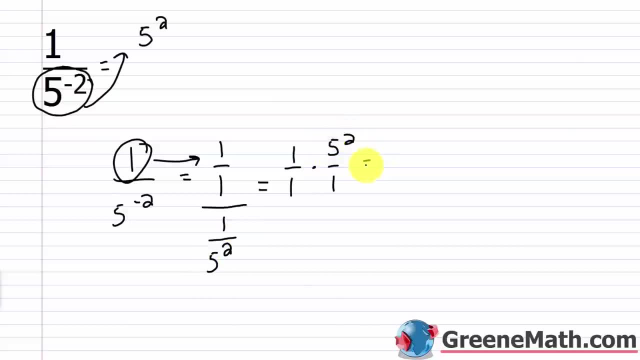 The reciprocal of this guy, which would be 5 squared over 1. At the end of the day, it's 1 times 5 squared, or 5 squared, over 1, which is just 5 squared. So again, the shortcut to that 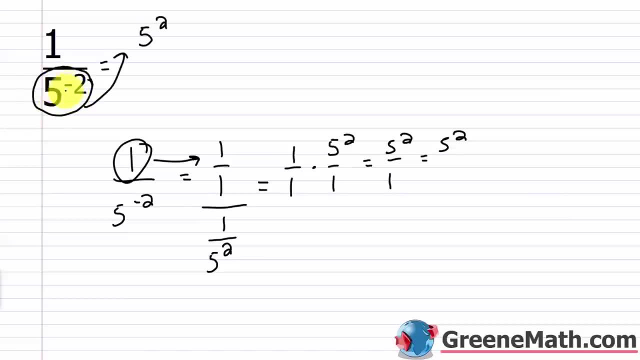 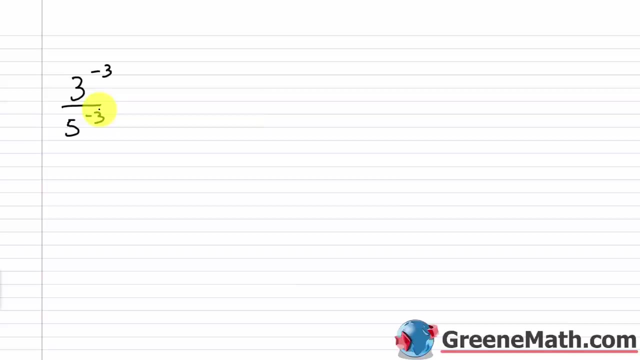 process is you're going to take the number from the denominator that's raised to a negative power, bring it into the numerator, and then you're going to take that exponent that's negative, and you're going to make it positive. Let's say I came across a problem like 3 to the power of negative 3 over 5 to the power of negative 3. So what does that mean? It means that I'm going to equal to. So the shortcut is to take what's in the numerator here, bring it into the denominator. 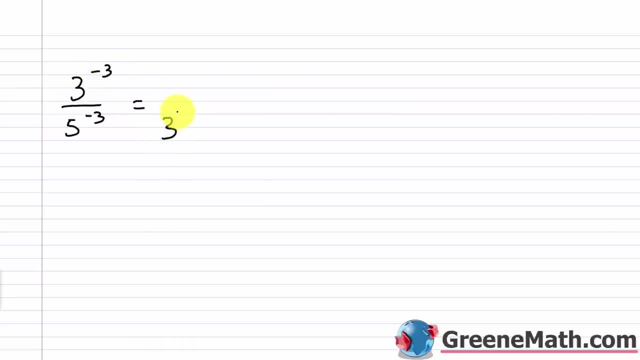 So 3 goes into the denominator. Instead of the exponent being negative, it's now going to be positive. And then this 5 here is in the denominator, bring it into the numerator. 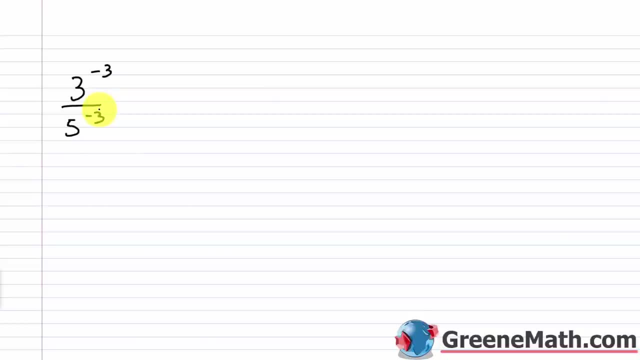 Let's say I came across a problem like three to the power of negative three, over five to the power of negative three. So what is this equal to? So the shortcut is to take what's in the numerator here, bring it into the denominator. 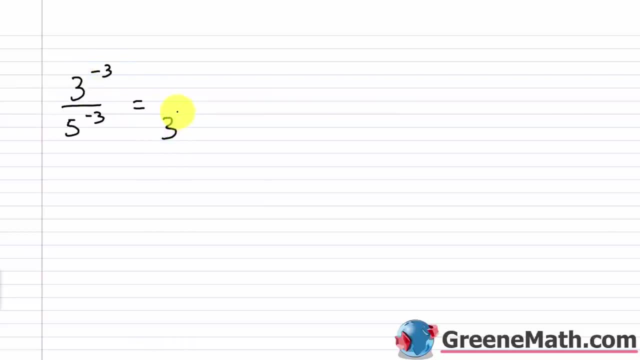 So three goes into the denominator. Instead of the exponent being negative, it's now gonna be positive. And then this five here is in the denominator. bring it into the numerator. Instead of the exponent being negative, make it positive. So this becomes five cubed over three cubed. 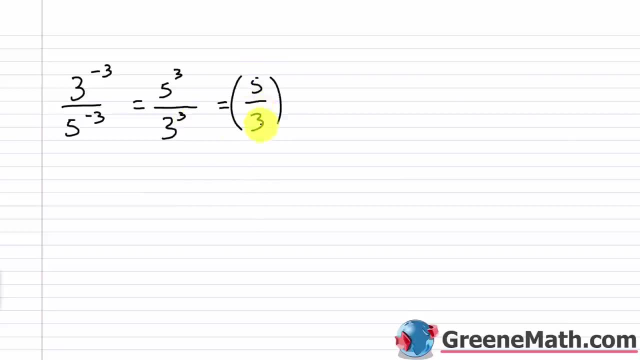 or I could write it as five over three, that amount cubed. Now if you wanna go about it the slow way, you can certainly do that. So three to the power of negative three is one over three cubed, And this is over. we have five to the power of negative three. 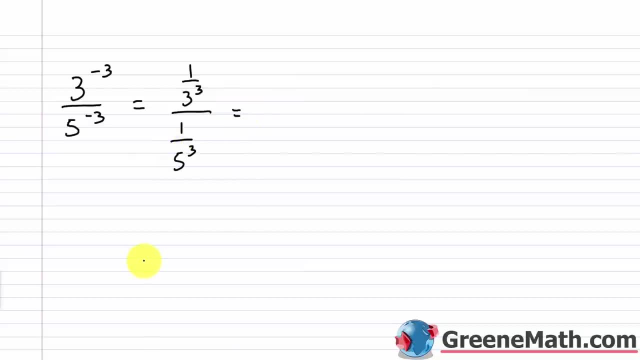 which is one over five cubed. We know how to divide fractions. The first one stays the same, So one over three cubed. We're gonna multiply this by the reciprocal of one over five cubed, which is five cubed over one. 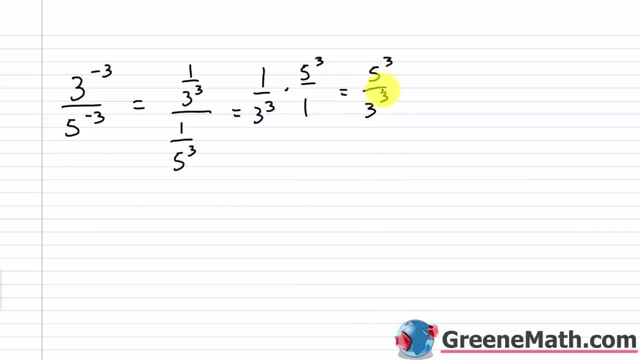 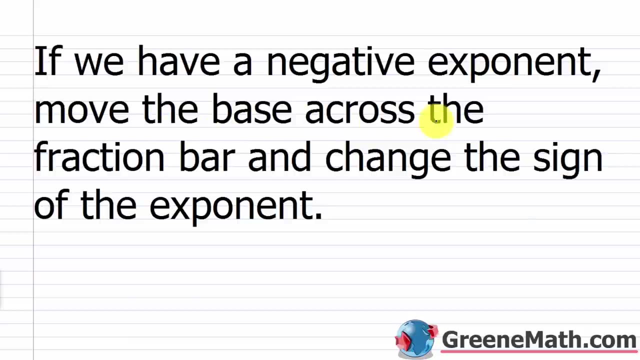 Of course we get five cubed over three cubed. So that leads us to this little simple rule here: If we have a negative exponent, move the base across the fraction bar and change the sign of the exponent. So in more mathy terms, 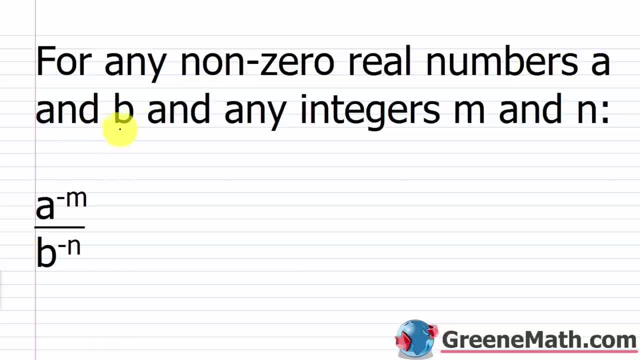 for any non-zero real numbers, A and B- and any integers- M and N- we can set up this: A to the power of negative M over B to the power of negative N is gonna be equal to. I would take this B and bring it into the numerator. 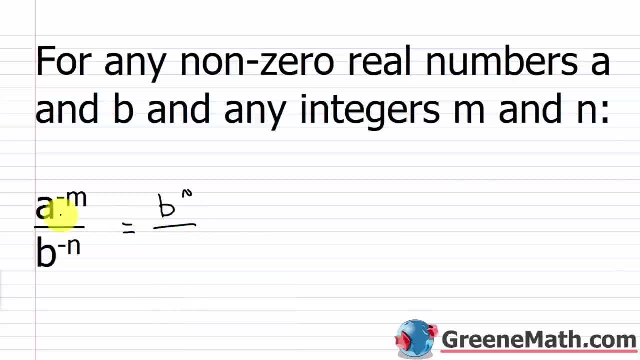 and raise it to a positive N, put it over A, which is gonna go into the denominator, and raise it to a positive M. So as an example, let's say I had something like I don't know. three to the power of negative six. 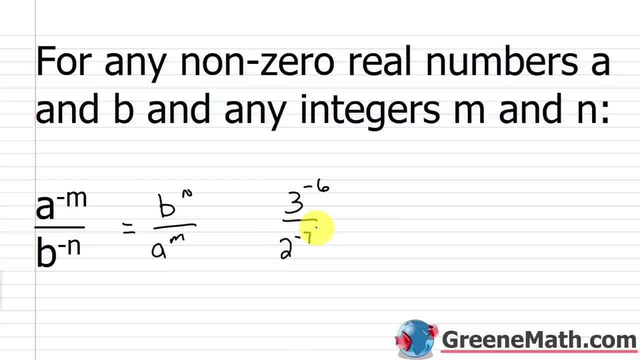 over two to the power of negative seven. All I need to do is take two, bring it into the numerator and make the exponent positive. So this is two to the seventh up here. Take three, bring it into the denominator, make the exponent positive. 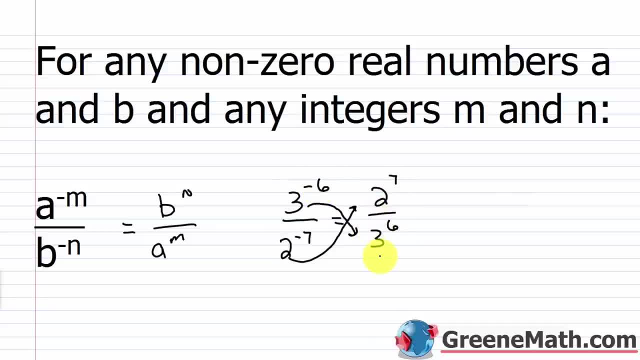 So this would be two to the seventh over three to the sixth. So again, if we have a negative exponent, move the base across the fraction bar. So that's why I move this two across the fraction bar, So from the denominator into the numerator. 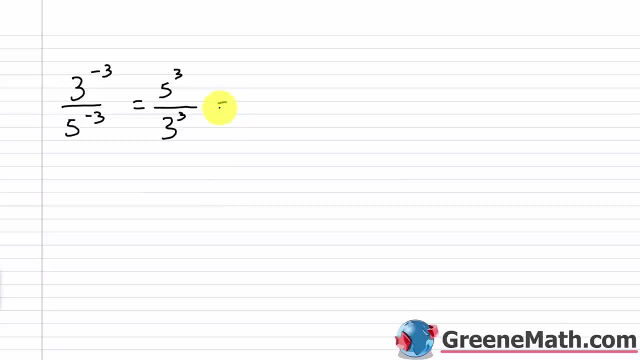 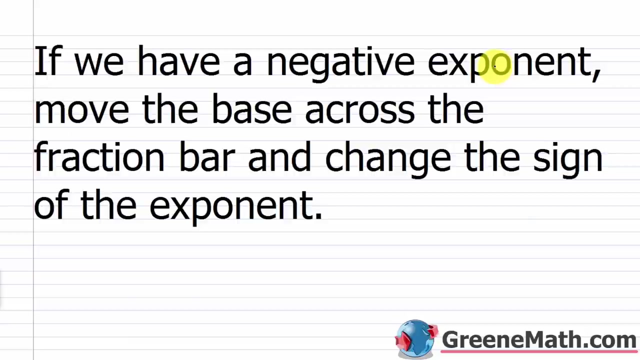 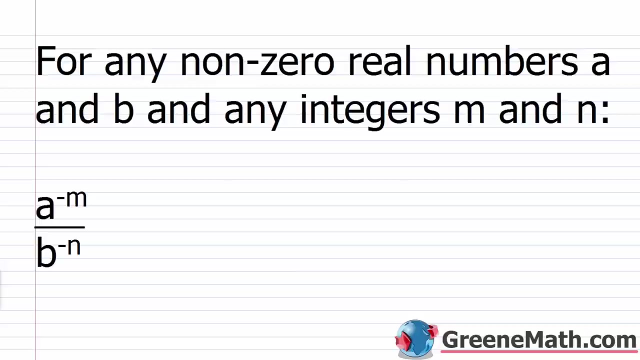 Instead of the exponent being negative, make it positive. So this becomes 5 cubed over 3 cubed, or I could write it as 5 over 3, that amount cubed. Now, if you want to go about it the slow way, you can start with the denominator. So I'm going to take the denominator, and I'm going to take the So 3 to the power of negative 3 is 1 over 3 cubed. And this is over, we have 5 to the power of negative 3, which is 1 over 5 cubed. We know how to divide fractions. The first one stays the same. So 1 over 3 cubed. We're going to multiply this by the reciprocal of 1 over 5 cubed, which is 5 cubed over 1. Of course, we get 5 cubed over 3 cubed. So that leads us to this little simple rule here. If we have a negative 3 to the power of negative 3 over 3 cubed, we're going to multiply a negative exponent, move the base across the fraction bar, and change the sign of the exponent. So in more mathy terms, for any non-zero real numbers a and b, and any integers m and n, we can set up this a to the power of negative m over b to the power of negative n is going to be equal to, I would take this b and bring it into the numerator and raise it to a positive n, put it over a, which is going to go into the denominator, and raise it to a positive m. 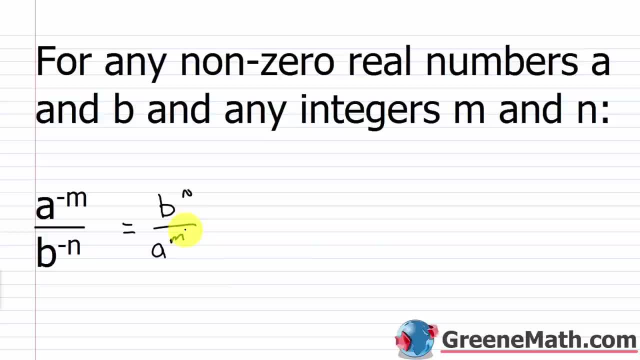 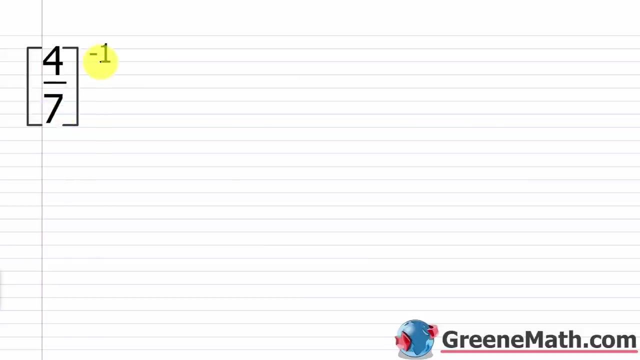 So as an example, let's say I had something like, I don't know, 3 to the power of negative 6 over 2 to the power of negative 7. All I need to do is take 2, bring it into the numerator, and make the exponent positive. So this is 2 to the 7th up here. Take 3, bring it into the denominator, make the exponent positive. And then I'm going to take the denominator, and put it over positive. So this would be 2 to the seventh over 3 to the sixth. So again, if we have a negative exponent, move the base across the fraction bar. So that's why I move this two across the fraction bar. So from the denominator into the numerator, see how it crosses above the fraction bar and then just change the sign of the exponent. So it was negative and now it's positive. I did the same thing here. I drag this below the fraction bar. It was negative, was negative, and now it's positive. So let's look at some quick examples here. We have 4 sevenths and this is raised to negative 1. So using our rules from our last lesson, we know we can write this as 4 to the power of negative 1 over 7 to the power of negative 1. And then what we just learned is we can take this 4 and drag it down here. Raises the power of positive 1. We can take this 7 to the power of negative 1 and drag it down here. Raises the power of positive 1. We can and drag it up here, raise it to the power of positive 1. So this is 7 over 4. It's just 7 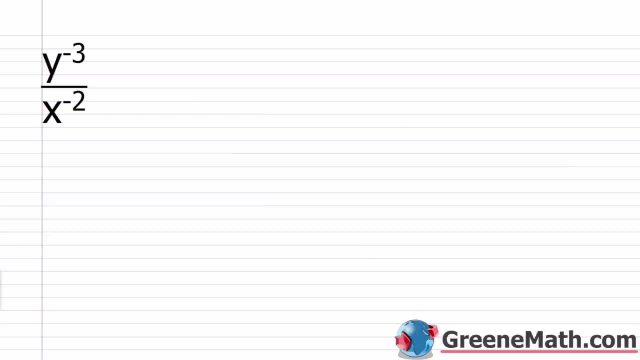 fourths. And the same goes when you're working with some variables. So for y to the power of negative 3 over x to the power of negative 2, this variable x is going to come up into the numerator, and I'm going to now raise it to positive 2. So that's x squared now. This y is going to go into the denominator, and I'm going to raise it to positive 3. So I get x squared over 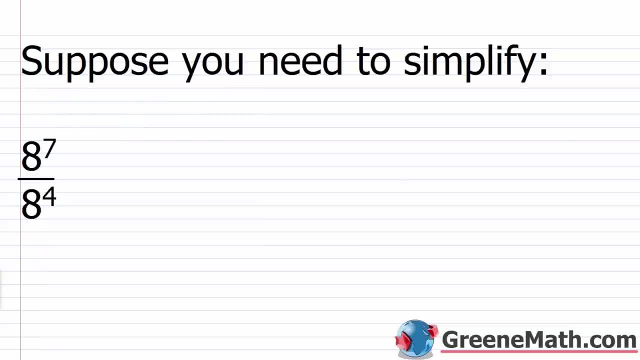 y cubed. Okay, so now let's talk about the last rule that we're going to learn, 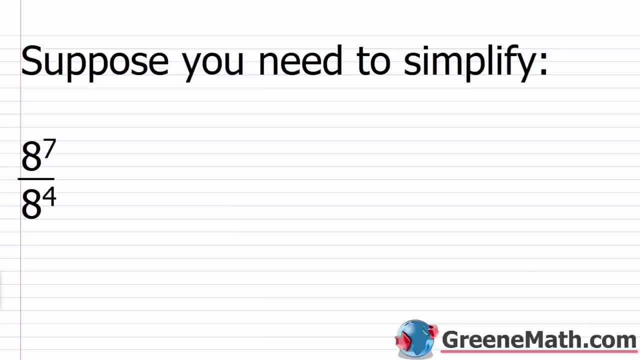 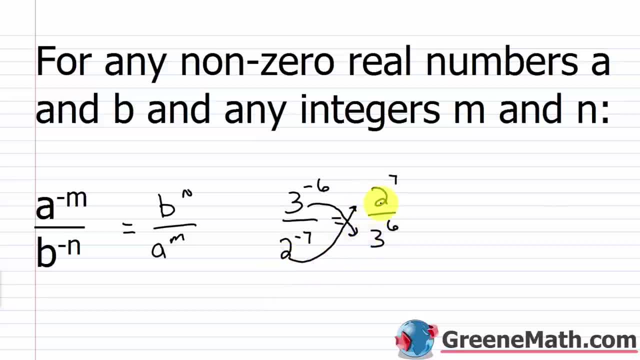 See how it crosses above the fraction bar and then just change the sign of the exponent. So it was negative and now it's positive. I did the same thing here. I dragged this below the fraction bar, It was negative, was negative and now it's positive. 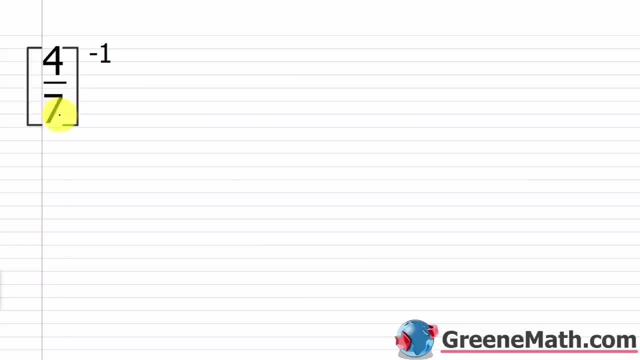 So let's look at some quick examples. here We have four sevenths and this is raised to negative one. So using our rules from our last lesson, we know we can write this as four to the power of negative one, over seven to the power of negative one. 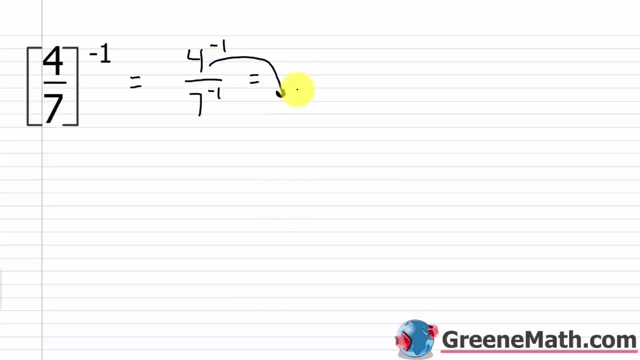 And then what we just learned is we can take this four and drag it down here, raise it to the power of positive one. We can take this seven and drag it up here, raise it to the power of positive one. So this is seven over four, just seven fourths. 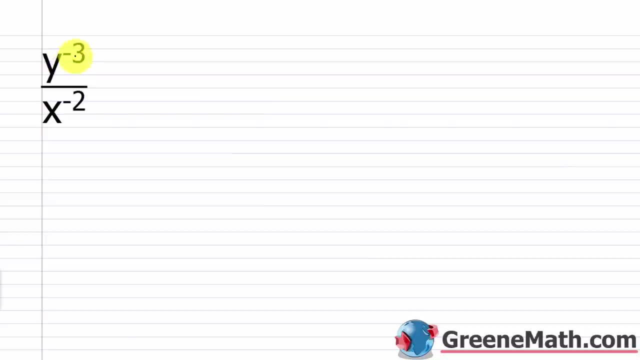 And the same goes when you're working with some variables. So for Y to the power of negative three or X to the power of negative two, this variable X is going to come up into the numerator. I'm going to now raise it to positive two. 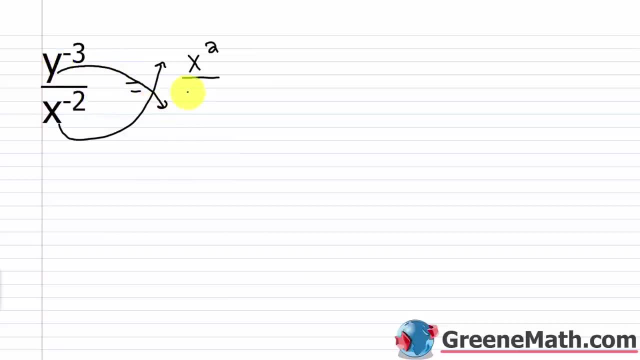 So that's X squared. Now this Y is going to go into the denominator and I'm going to raise it to positive three. So I get X squared over Y cubed. OK, so now let's talk about the last rule that we're going to learn. 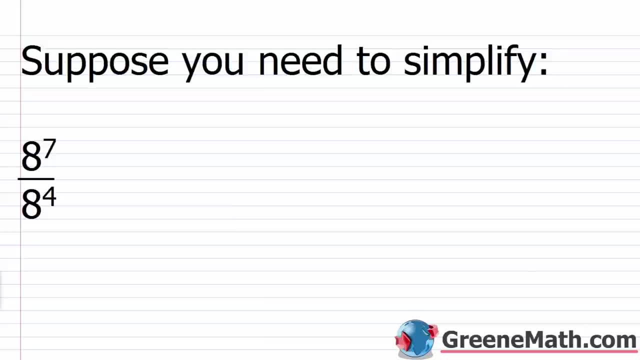 And it's known as the quotient rule for exponents. So I want you to suppose that you need to simplify something like eight to the seventh power over eight to the fourth power. So with the knowledge we already have learned, we could take eight to the seventh power. 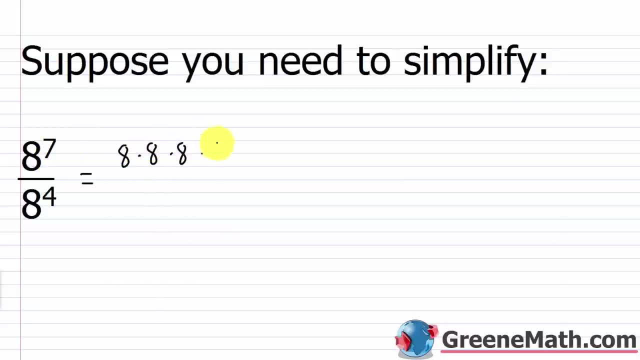 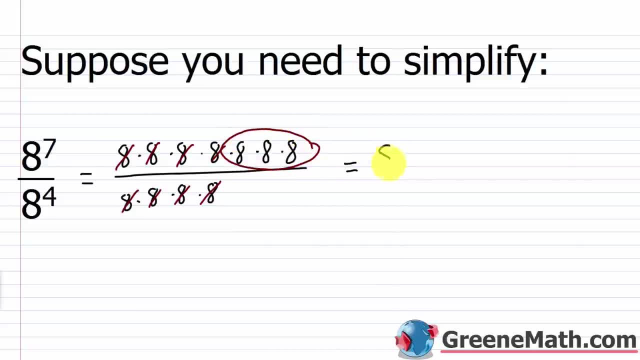 And I'm left with three factors of eight or eight to the third power. But how can we do this more quickly? Like I realize that the exponent that I have right here in the top minus the exponent that I have right here on the bottom gave me the ending exponent. 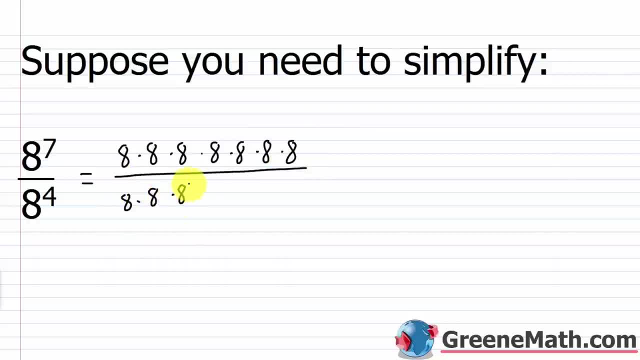 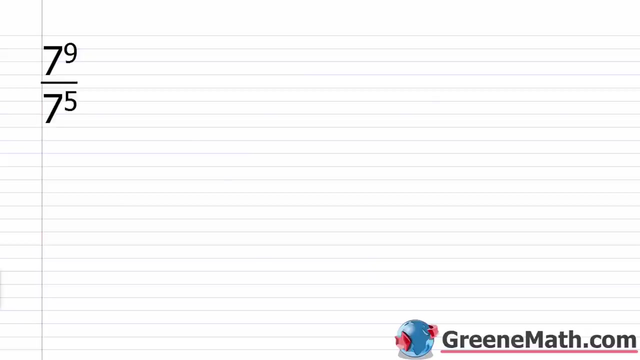 Let's see. Over 8 times 8 times 8 times 8. All right. We can cancel common factors between numerator and denominator. We cancel this with this, this with this, this with this, and this with this, and I'm left with three factors of 8 or 8 to the 3rd power. But how can we do this more quickly? Like I realized that the exponent that I have right here in the top minus the exponent that I have right here on the bottom gave me the ending. So I could have started out with saying, okay, I have 7 factors of 8, and I'm going to be canceling away 4 factors of 8. So that's going to leave me with 7 minus 4 or 3 factors of 8. So if I saw something like 7 to the 9th power over 7 to the 5th power, you guessed it. I can take this number right here, this 9, and I can subtract away this number right here, this 5, and I would get 7 to the 4th power, right? And to see that once more, again, if I write out 9 factors of 8, I'm going to have 9 factors of 7, 1, 2, 3, 4, 5, 6, 7, 8, 9, over 5 factors, 1, 2, 3, 4, 5. What's going to happen is I'm going to end up canceling 5 factors of 7 here. In other words, if I think about this using the exponents, I'm starting out with 9, and I'm subtracting away 5, I'm going to end up with 4, right? Cancel this, cancel this, cancel this. 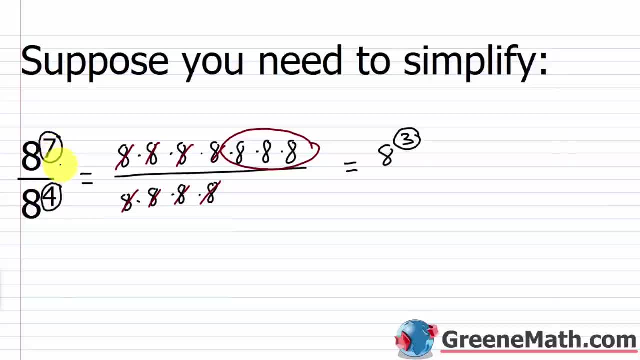 So I could have started out with saying: OK, I have seven factors of eight and I'm going to be canceling away four factors of eight. So that's going to leave me with seven minus four or three factors of eight. So if I saw something like seven to the ninth power over seven to the fifth power, 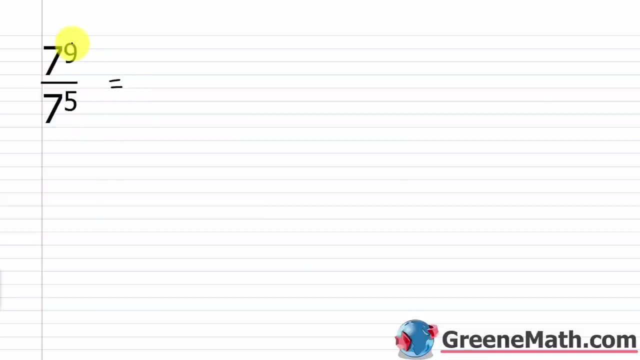 you guessed it. I can take this number right here, this nine, and I can subtract away this number right here, this five, and I would get seven to the fourth power Right. And to see that once more again, if I write out nine factors of seven, 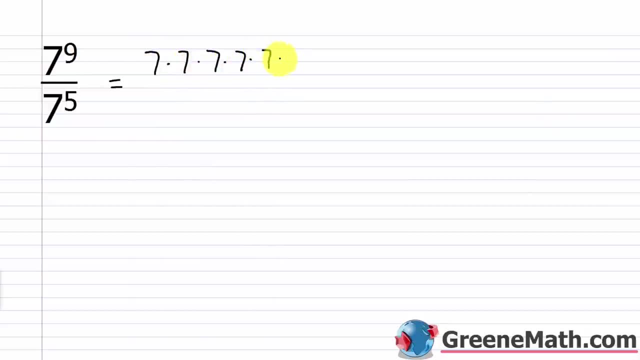 one, two, three, four, five, six, seven, eight, nine Over five factors: one, two, three, four, five. It's going to happen is I'm going to end up canceling five factors of seven here. 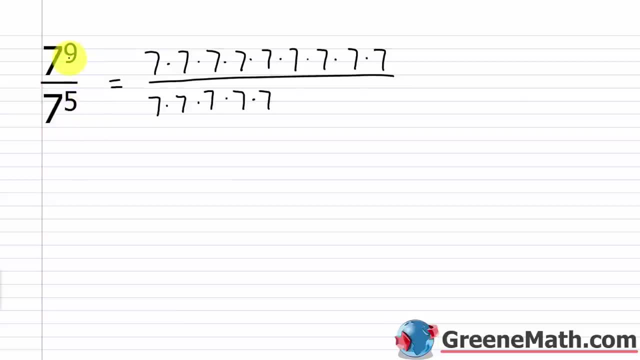 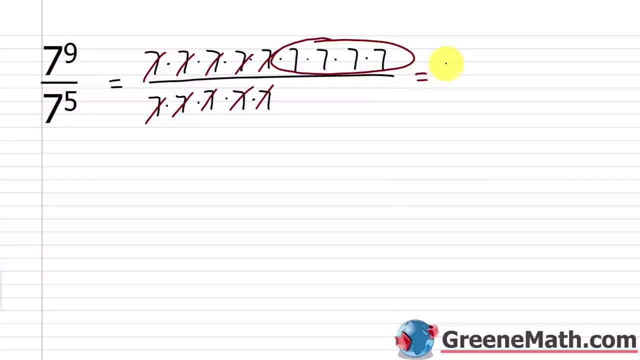 This is what I'm left with. I'm left with four factors of seven, or seven to the fourth power. So So this leads us to the following rule: for any non-zero real number, A, and any integers- M and N, We want to keep the base the same and subtract M minus N. 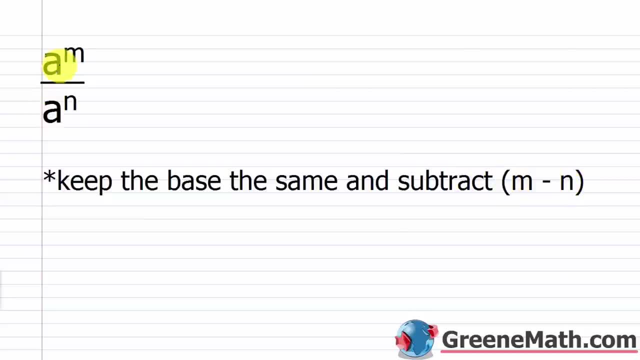 So, in other words, if I have the same base here, the same non-zero real number, and they're involved in a division that looks like this, all I need to do is keep the base the same. So I would keep A the same and I would subtract the exponents. 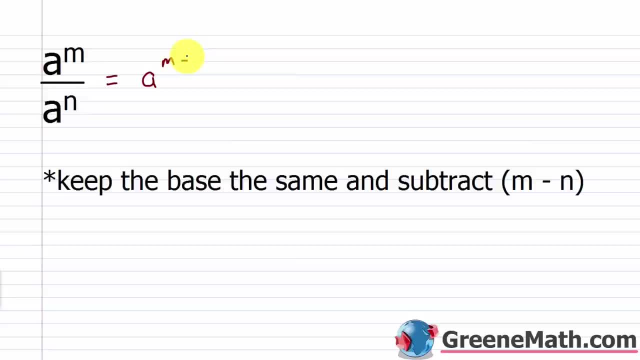 I would take the one in the numerator Which is M and I would subtract away the one in the denominator which is N. So for five, ninths, over five cubed again, this is the same base. So I write five. So I take my exponent, the numerator which is nine. 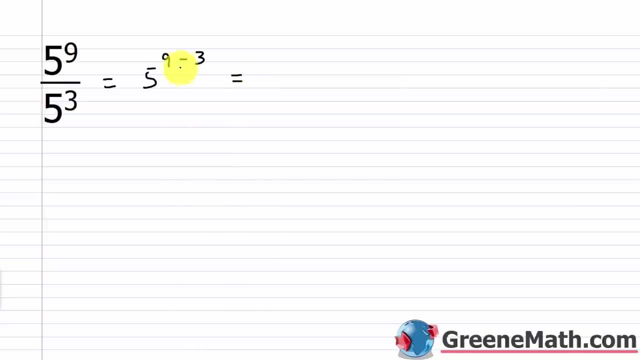 And I subtract away my exponent the denominator, which is three and nine minus three is six, So this is five to the sixth power. Again, you can prove that to yourself. You can write out nine factors of five And then underneath you can write out three factors of five and you can cancel three factors of five away. 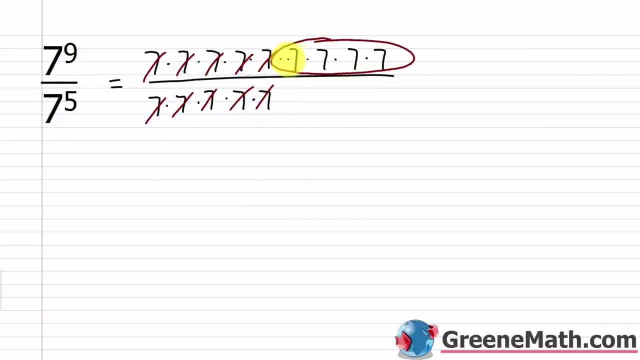 Cancel this and cancel this. This is what I'm left with. I'm left with 4 factors of 7 or 7 to the 4th power. So this leads us to the following rule. For any non-zero real number a and any integers m and n, we want to keep the base the same and subtract m minus n. So in other words, if I have the same base here, the same non-zero real number, and they're involved in a division that looks like this, all I need to do is keep the base the same. So I would keep a the same and I would subtract the exponents. I would take the one in the numerator, which is m, and I would subtract away the one in the denominator, which is n. So for 5 ninths over 5 cubed, again, this is the same base. So I write 5. So I take my exponent in the numerator, which is 9, and I subtract away my exponent in the denominator, which is 3. And 9 minus 3 is 6. So this is 5 to the 6th power. Again, you can prove that to yourself. 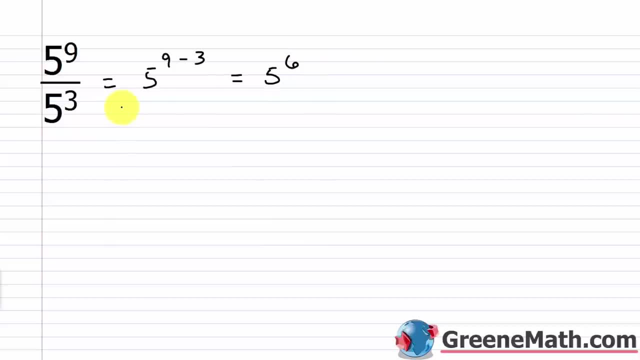 You can write out 9 factors of 5. And then underneath, you can write out 3 factors of 5. And you can cancel 3 factors of 5 away from the problem you create there. And you're going to end 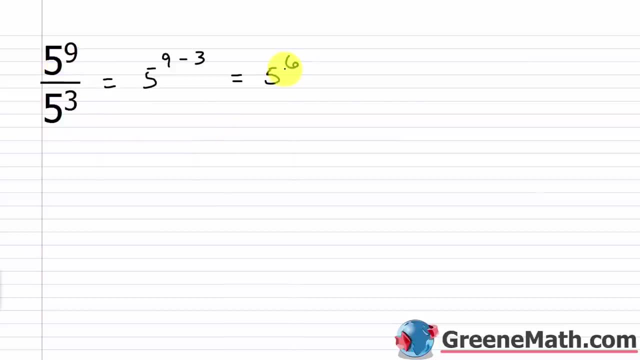 up with 6 factors of 5, which again is our result. All right. Here we have x to the 4th power y 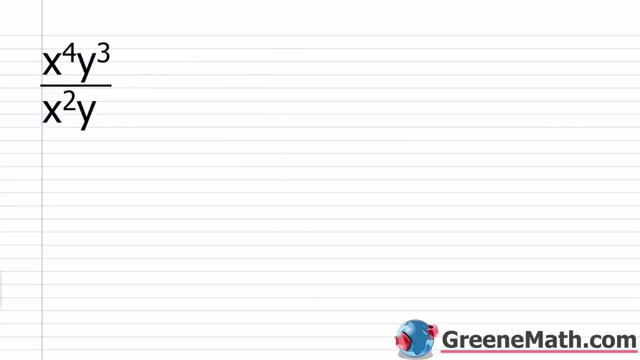 cubed over x squared y. So for x to the 4th power over x squared, I would keep the base x the same. 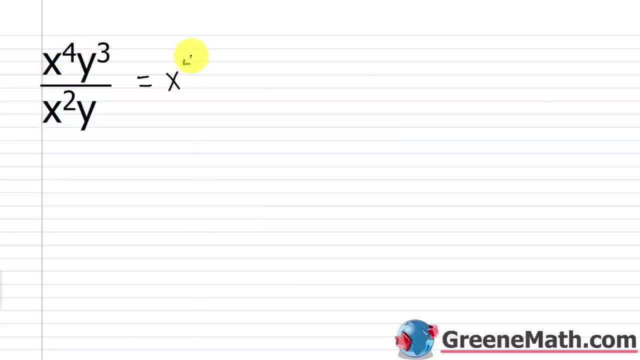 Then I would subtract exponents. So I would take the exponent in the numerator, which is 4. Subtract away the exponent in the denominator, which is 2. And then I have y cubed 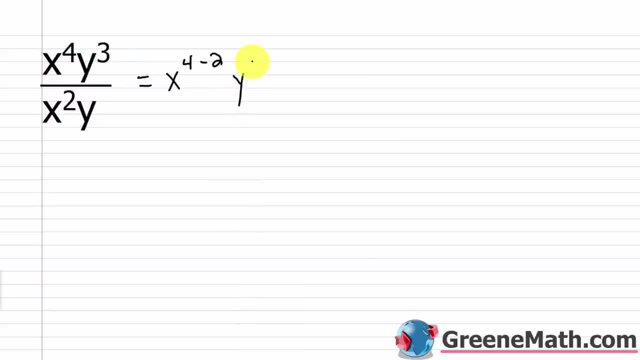 over y. So I'm going to put y down, keep the base the same. And then I'll have 3 minus. This exponent will be 1. So 3 minus 1. So this equals x squared. 4 minus 2 is 2. Times y squared also. 3 minus 1 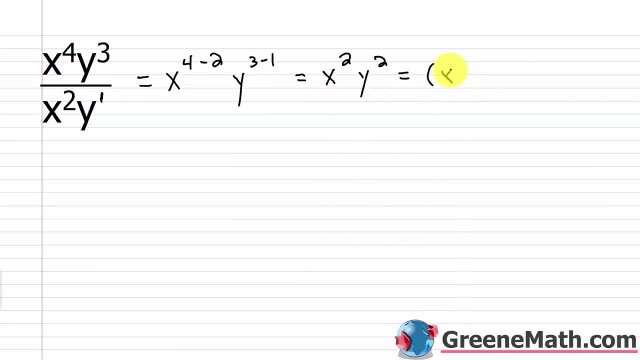 is 2. So you could write x squared y squared, or you could write xy, this inside of parentheses, squared. So even when negative exponents are in the denominator, you can write x squared y squared. 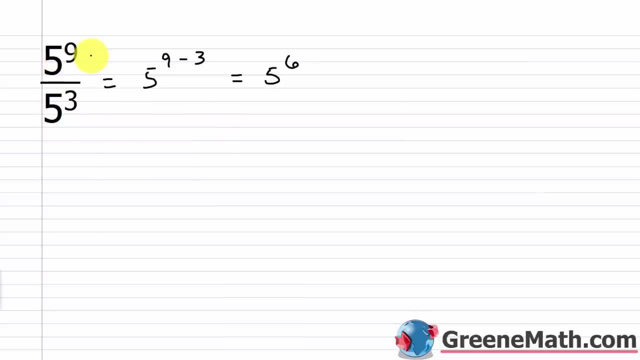 From the problem you create there, you're going to end up with six factors of five, which again is our result. All right, here we have X to the fourth power, Y cubed over X squared Y. So for X to the fourth power over X squared, I would keep the base X the same. 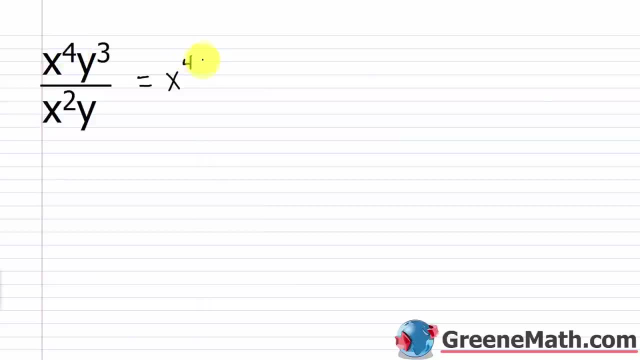 Then I would subtract exponents. So I'll take the exponent, the numerator, which is four, subtract away the exponent, the denominator, which is two, And then I have Y cubed over Y, So I'm going to put Y down. 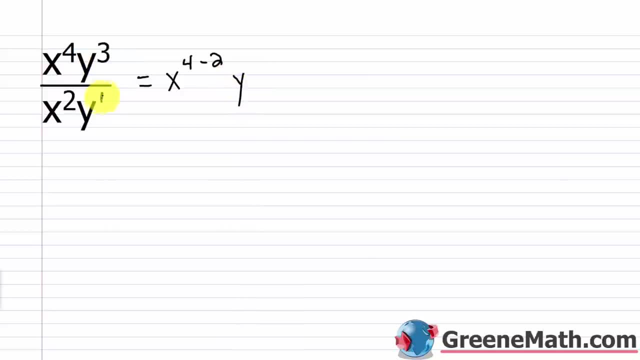 Keep the base the same, And then I'll have three minus this exponent will be one, So three minus one. So this equals X squared. four minus two is two times Y squared. also, three minus one is two, So you could write X squared, Y squared, or you could write X, Y- this inside of parentheses- squared. 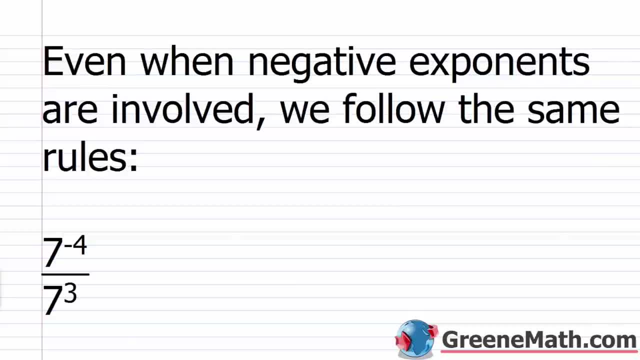 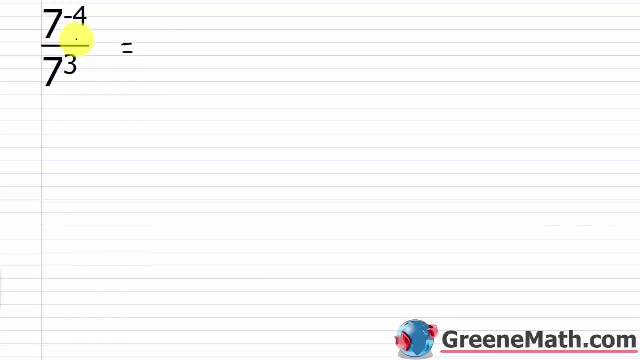 So even when negative exponents are involved, we follow the same rules. So we have seven to the power of negative four over seven cubed. So what I'm going to do is I'm going to keep that base. So I'm going to keep seven, the same. 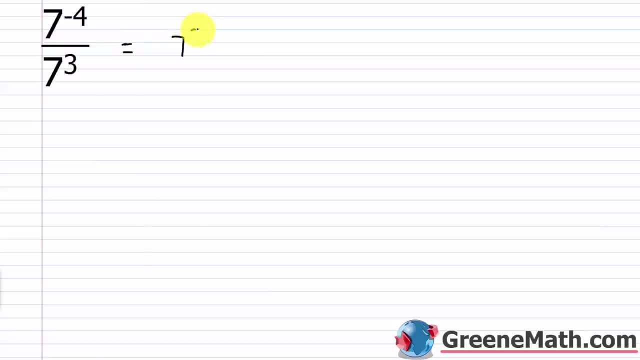 And then I'm going to subtract the exponent in the numerator, which is negative four, minus the exponent in the denominator, which is three. So this gives me seven to the power of negative four minus three, which is seven. to the power of negative seven, which we write as one over seven, to the seventh power. 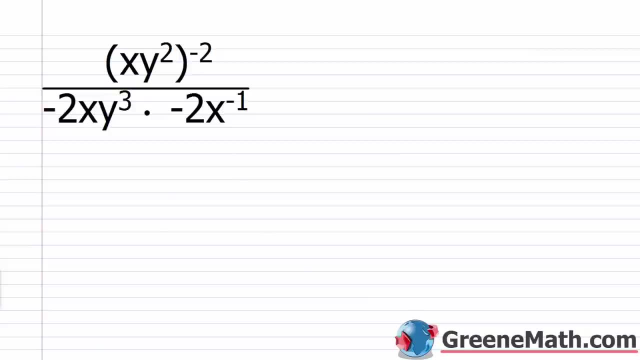 All right, let's take a look at some practice problems to kind of wrap up the lesson. So we have X- Y squared- This is in parentheses- and it's raised to the power of negative two. Then this is over. we have negative two times X, Y cubed times. negative two times X to the power of negative one. 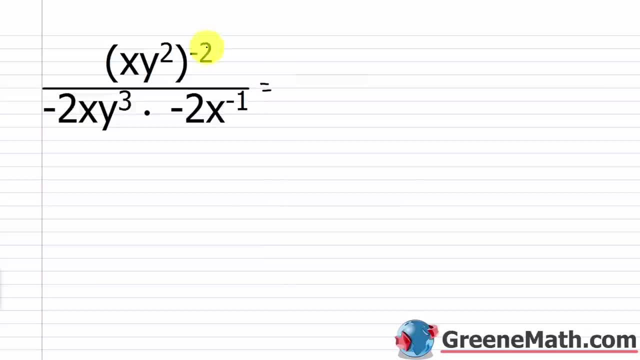 So let's start out in the numerator. Let's use our power to power rule to simplify. So we have X raised to the power of negative two, So that's X to the power of negative two. And then we have Y squared, that's raised to the power of negative two. 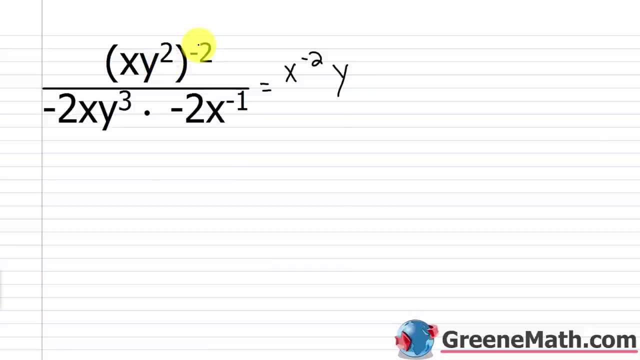 So Y stays the same. We multiply the exponents two times negative two is negative four In the denominator. I have a negative two, I have an X, I have a Y cubed and I'm multiplying this by another negative two and X raised to the power of negative one. 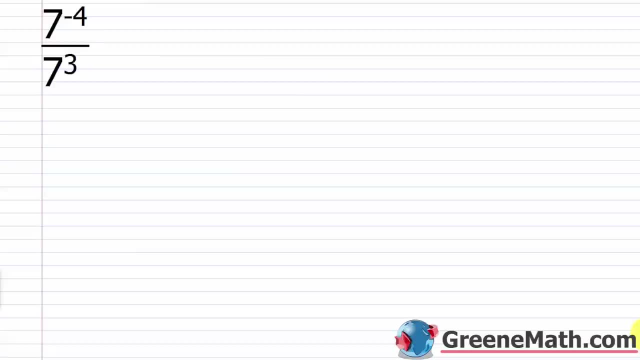 So we have 7 to the power of negative 4 over 7 cubed. So what I'm going to do is I'm going to keep that base 7 the same. And then I'm going to subtract the exponent in the numerator, which is negative 4, minus the exponent in the denominator, which is 3. So this gives me 7 to the power of negative 4 minus 3, which is 7 to the power of negative 7, which we write as 1 over 7 to the 7th power. 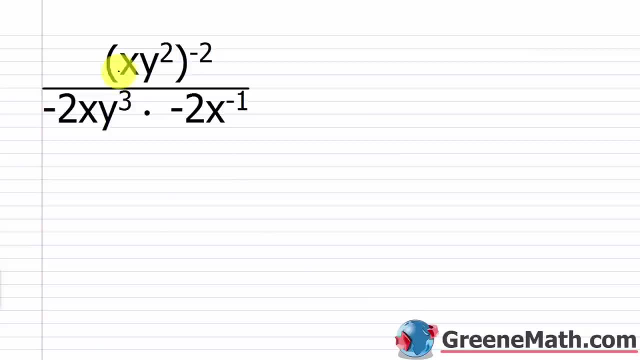 So let's look at some practice problems to kind of wrap up the lesson. So we have xy squared, this is in parentheses and it's raised to the power of negative 2. Then this is over, we have negative 2 times xy cubed times negative 2 times x to the power of negative 1. So let's start out in the numerator. Let's use our power to power rule to simplify. So we have x raised to the power of negative 2. So that's x to the power of negative 2. And then we have y squared, that's raised to the power of negative 2. So y stays the same, we multiply the exponents. 2 times negative 2 is negative 4. In the denominator I have a negative 2, I have an x, I have a y cubed, and I'm multiplying this by another negative 2, and x raised to the power of negative 1. Now before I simplify any further between numerator and denominator, let me simplify this denominator. 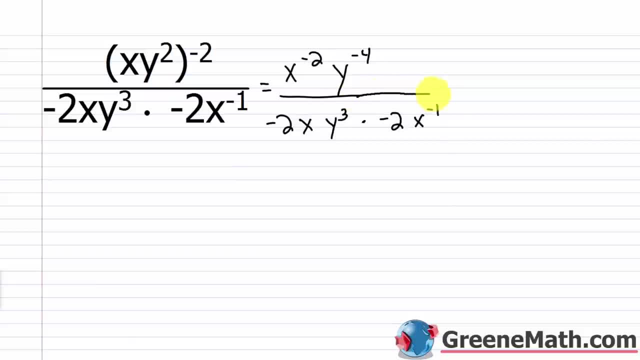 Now, before I simplify any further between numerator and denominator, let me simplify this denominator here. Let me just erase this and make a new line. So negative two times negative two is four. Or if you want to kind of Keep with the spirit of exponents, I could write negative two inside of parenthesis, squared like that. 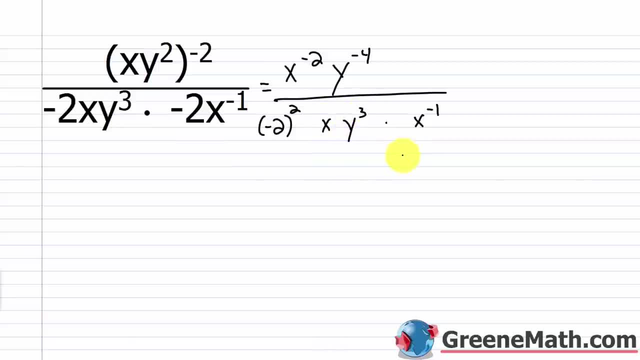 Then I have X, Y cubed, and we're multiplying this by X raised to the power of negative one. Now, this can be combined with this: X to the power of one times X to the power of negative one Is what Well remember. X to the power of negative one. 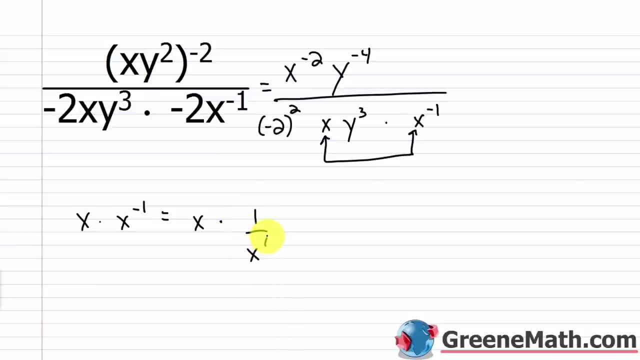 Is one over X to the first power. So really, what this becomes is X over X, which is one, And you can verify this using your product rule for exponents. This is X to the first power times X to the power of negative one. 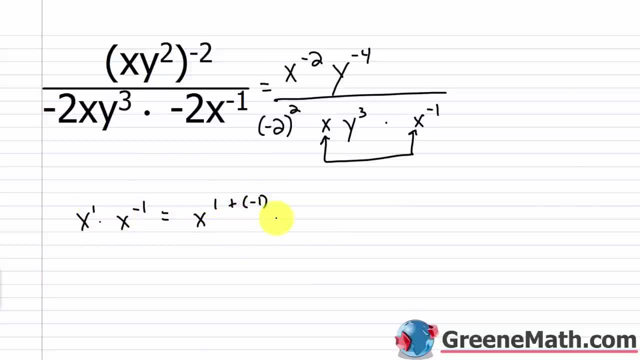 Well, this is X to the power of one, plus negative one, which equals X to the power of zero, which by definition is one. So essentially these two Would cancel out and you could just erase them. So I'm just left with this negative two, inside of parenthesis, squared. 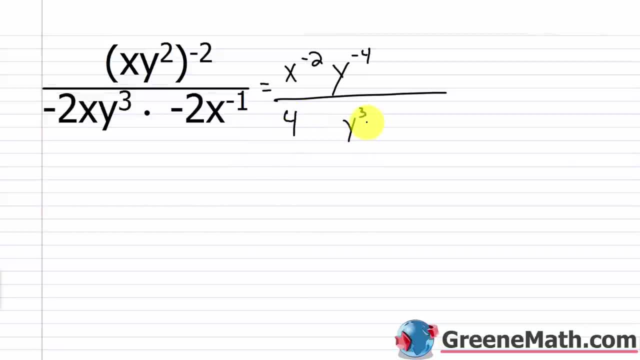 So I'm just going to go ahead and write as four times Y. cubed. Now to simplify this further: in the numerator I have X to the power of negative two, and then I have Y to the power of negative four. Now to simplify, I have a Y cubed down here. 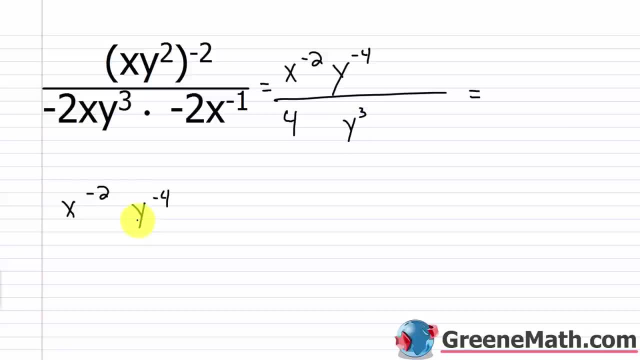 So again, the quotient rule for exponents tells me that same base. I can take that base. Keep it the same, which is Y, And I could subtract. take the exponent in the numerator which is negative four, subtract away the exponent of the denominator, which is three. 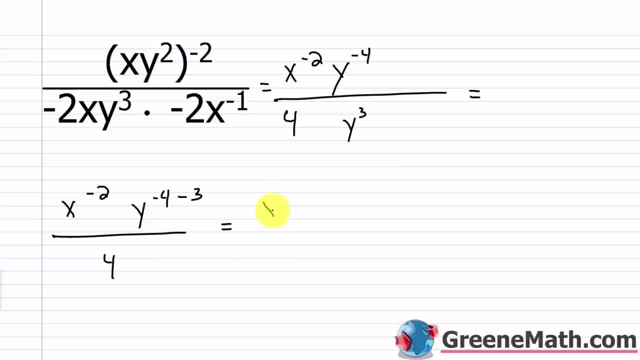 So then this is over four, And this equals X to the power of negative two times Y raised to the power of negative four minus three, which is negative seven. This is over four. So this is going to be equal to. These are both going to get moved down into the denominator. 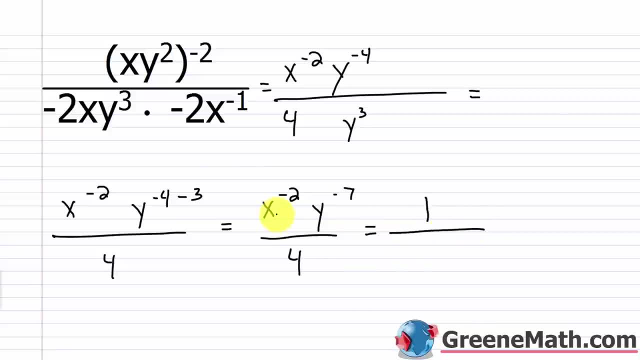 So I'm going to write the numerator as a one. This guy right here Again, like I just said, it's going to come down here, And so is this guy. So I have my four. that's going to stay the same. 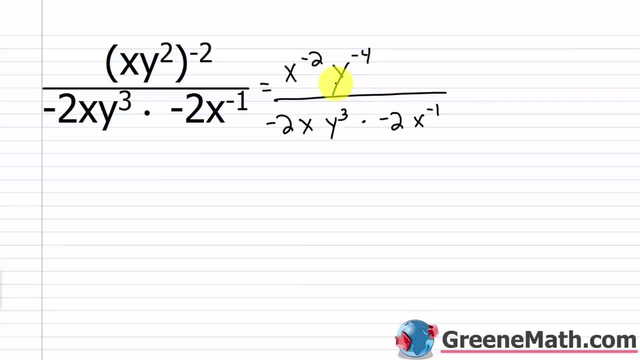 here let me just erase this and make a new line so negative 2 times negative 2 is 4 or if you want to kind of keep with the spirit of exponents I could write negative 2 inside of parentheses squared like that then I have x y cubed and we're multiplying this by x raised to the power of negative 1 now this can be combined with this x to the power of 1 times x to the power of negative 1 is what well remember x to the power of negative 1 is 1 over x to the first power so really what this becomes is x over x which is 1 and you can verify this using your product rule for exponents this is x to the first power times x to the power of negative 1 well this is x to the power of 1 plus negative 1 which equals x to the power of 0 which by definition is 1 so essentially these two would cancel out you could just erase them so I'm just left with this negative 2 inside of parentheses squared so I'm just going to go ahead and write as 4 times y cubed now to simplify this further in the numerator I have x to the power of negative 2 and then I have y to the power of negative 4 now to simplify I have a y cubed down here so again the quotient rule for exponents tells me that same base I can take that base keep it the same which is y and I can subtract take the exponent in the numerator which is 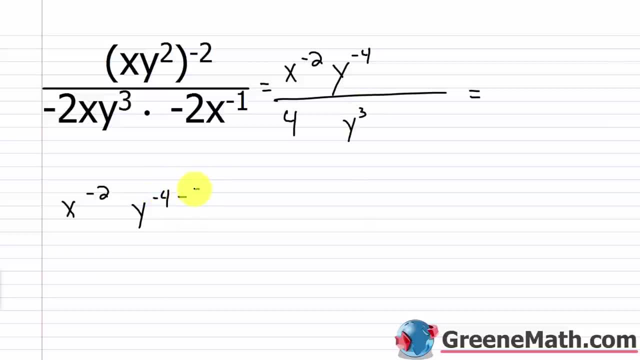 negative 4 subtract away the exponent in the denominator which is 3 so then this is over 4 and this equals x to the power of negative 2 times y raised to the power of negative 4 minus 3 which is negative 7 this is over 4 so this is going to be equal to these are both going to get moved into the denominator so I'm going to write the numerator as a 1 this guy right here again like I just said it's going to come down here and so is this guy so I have my 4 that's going to stay the same so when I drag this below the fraction bar the x stays the same but then the exponent is going to go from negative to positive then the y is going to go down there the exponent goes from negative to positive and because these two both went down there I'm going to write a 1 as my numerator so I'll put something like x squared y cubed times two x squared y to the power of negative 2 over y to the power of negative 2 and then everything's inside of brackets and it's raised to the power of 0 well the shortcut here is to remember that everything is raised to the power of 0 here anything raised to the power of 0 is 1 so you see that on a test you just put 1 but you can go through it and do the power to power rule for everything what's going to happen is every single thing in here is going to end up being raised to the power of 0 so you'll just 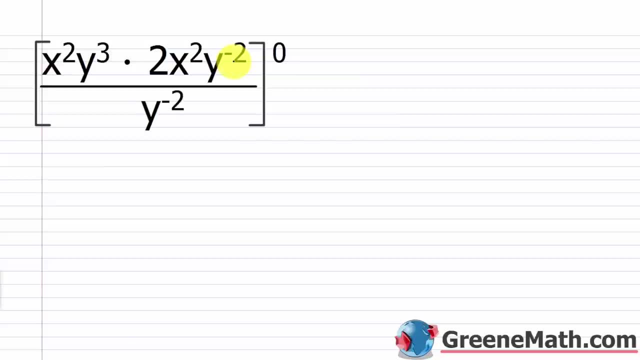 have 1 times 1 times 1 times 1. A bunch of 1's being multiplied by itself. And then down here 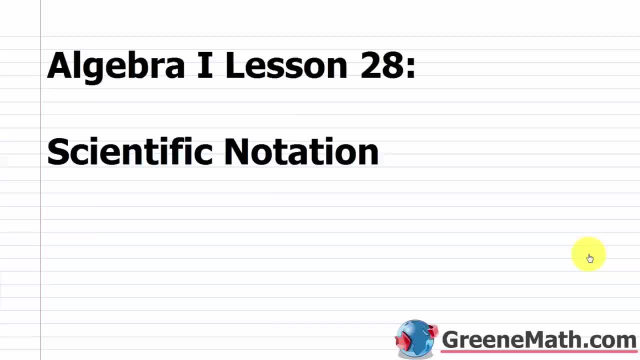 it'd be over 1. So you'd end up with just the number 1. Hello and welcome to Algebra 1 Lesson 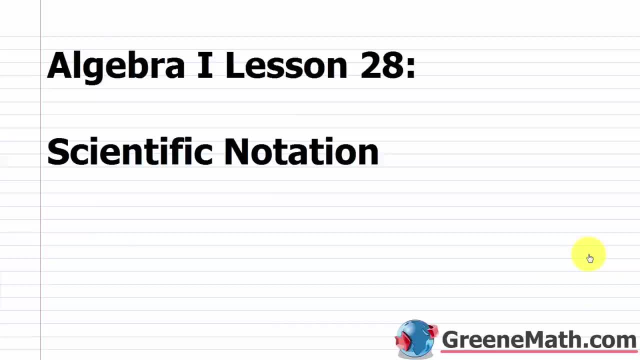 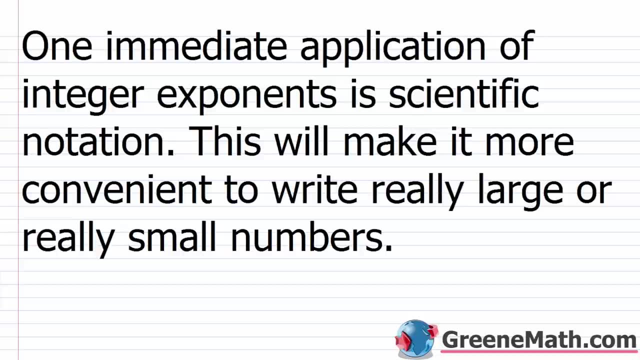 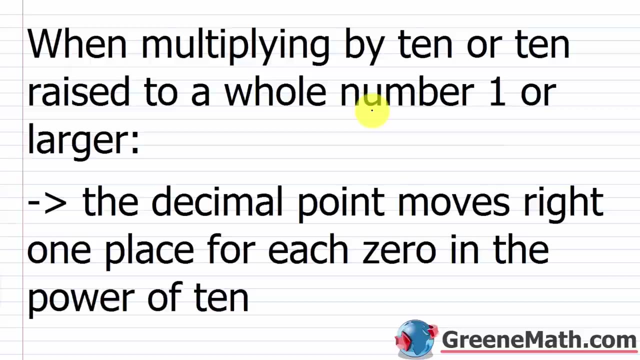 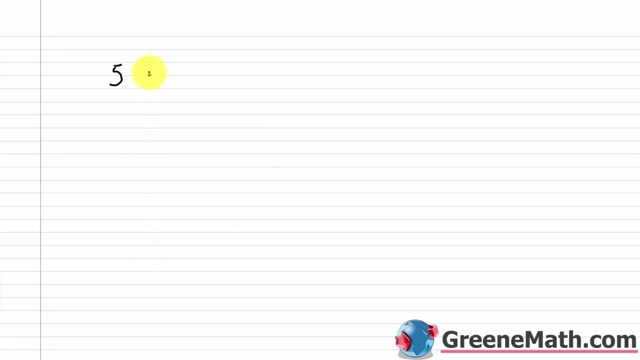 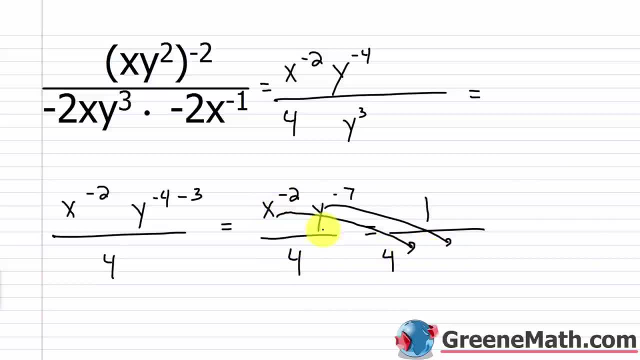 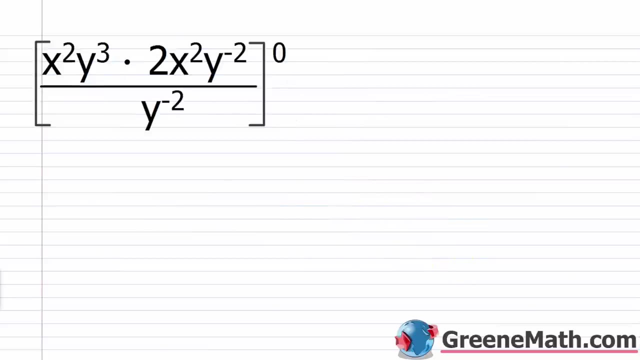 So when I drag this below the fraction bar, the X stays the same, But then the exponent is going to go from negative to positive, Then the Y is going to go down. there The exponent goes from negative to positive. And because these two both went down there, I'm going to write a one as my numerator about something like X squared Y, cubed times two. X squared Y to the power of negative two. 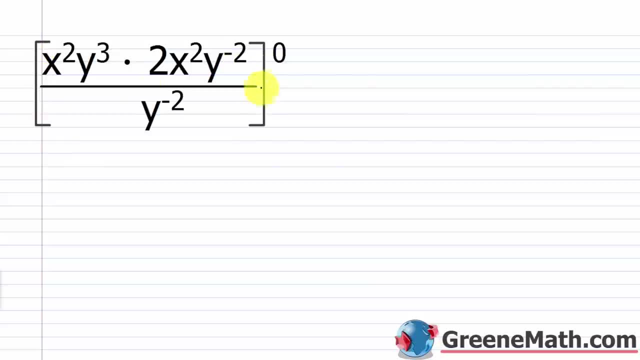 Over Y to the power of negative two, And then everything's inside of brackets and it's raised to the power of zero. Well, the shortcut here is to remember that everything is raised to the power of zero here. Anything raised to the power of zero is one. 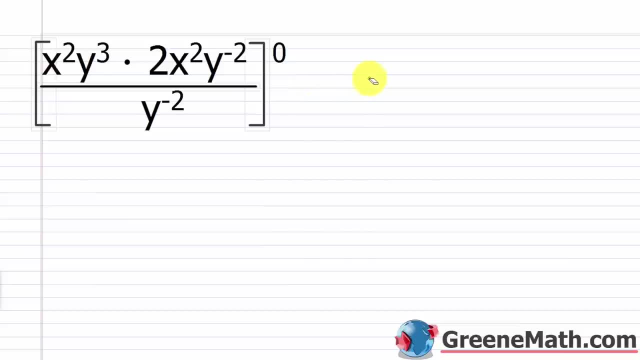 So you see that on a test you just put one, But you can go through it and do the power to power rule for everything. What's going to happen is every single thing in here is going to end up being raised to the power of zero. 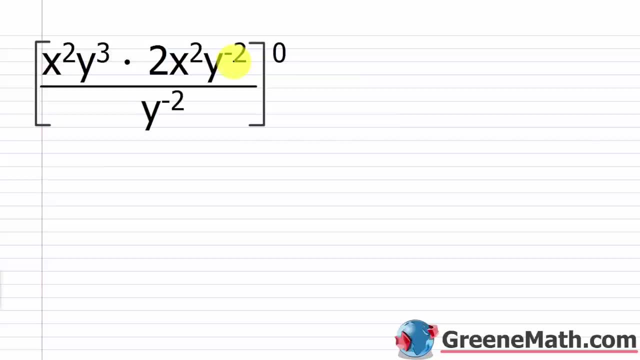 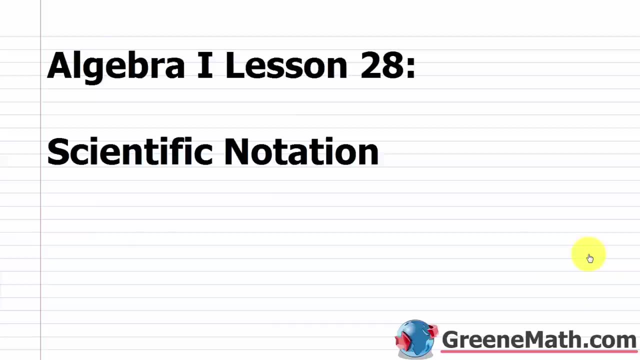 So you'll just have one times one times, one times one, to a bunch of ones being multiplied by itself, And then down here it'd be over one, So you'd end up with just the number one. Hello and welcome to Algebra 1, Lesson 28.. 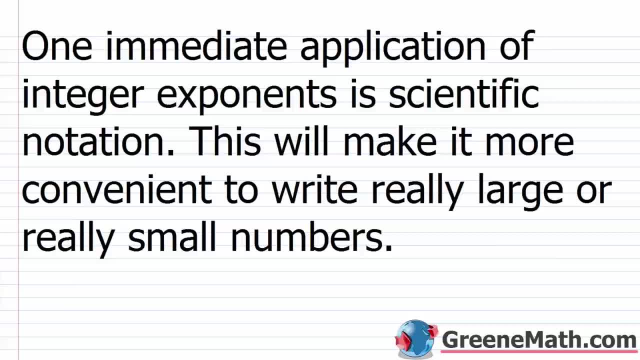 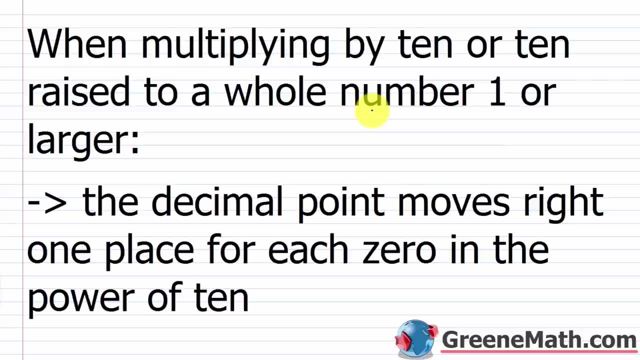 In this video we're going to learn about scientific notation. So one immediate application of integer exponents is scientific notation. This will make it more convenient to write really large or really small numbers. So before we get into scientific notation, I want to review some things from pre-algebra. 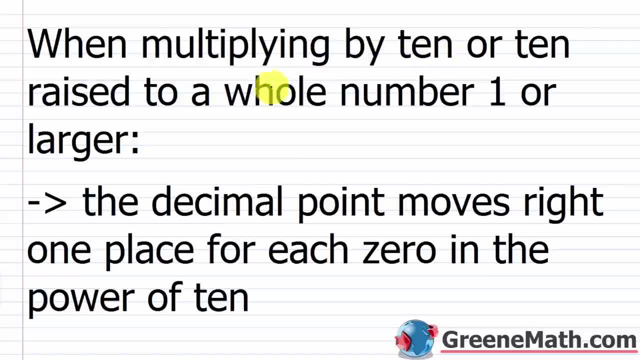 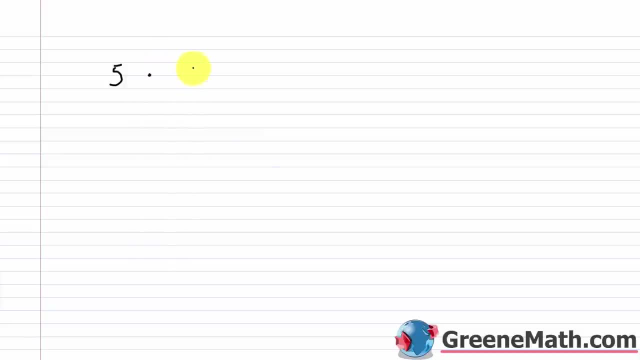 So the first thing is that when multiplying by 10, or 10 raised to a whole number, one or larger, the decimal point moves right one place for each zero in the power of 10.. So, for example, if I take, let's say, the number five and I was to multiply five by, let's say, 100.. 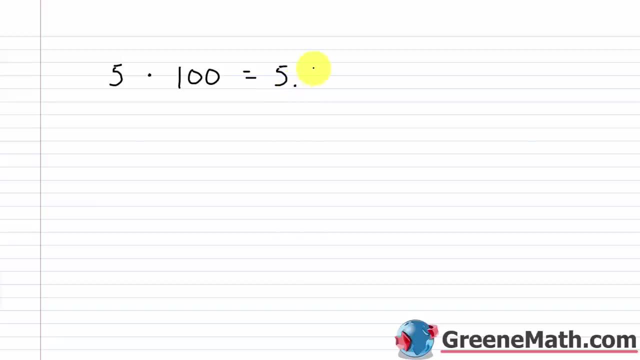 Well, this is equal to: I could just write five as five point zero, And I can move this decimal point one place to the right for every zero in this power of 10.. So there's two zeros Here, two zeros. So this would go: one, put another zero in there, two places to the right, and we'd end up with the number 500. 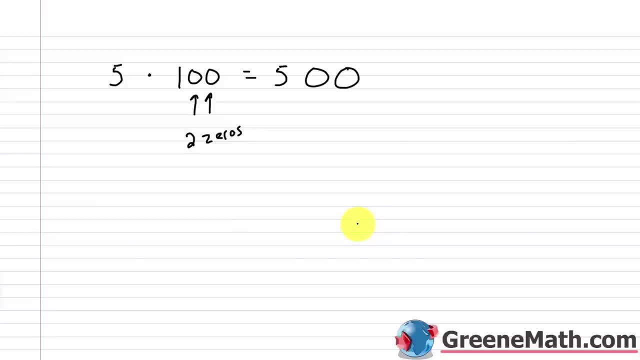 And we all know five times 100 is 500, but that's kind of another way you can do it. And you could also think about this as, let's say, five times I don't know. let's say we had 10,000. 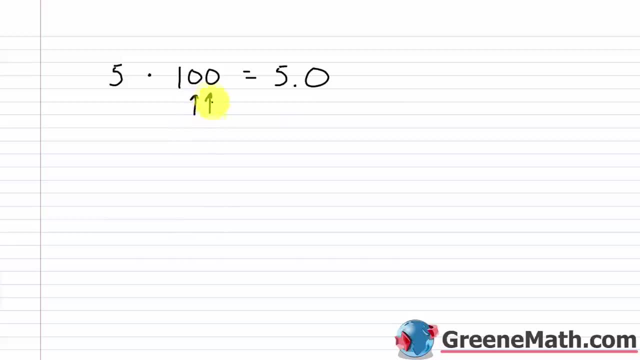 every zero in this power of 10. So there's two zeros here. Two zeros. So this would go 1, put another zero in there, two places to the right, and we'd end up with the number 500. And we all know 5 times 100 is 500, but that's kind of another way you can do it. And you could also think about this as let's say 5 times, I don't know, let's say we had 10,000. 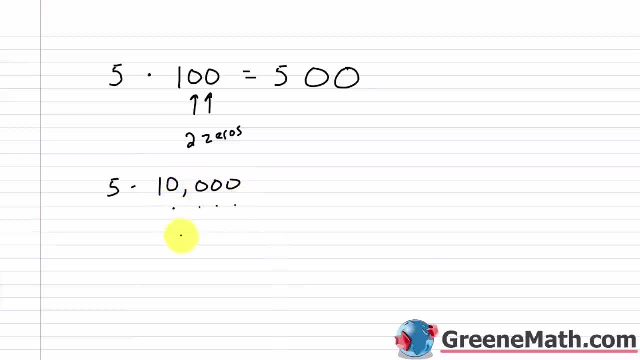 So there's 1, 2, 3, 4 zeros. So 4 zeros. So again, I could put equals 5.0. And I can move 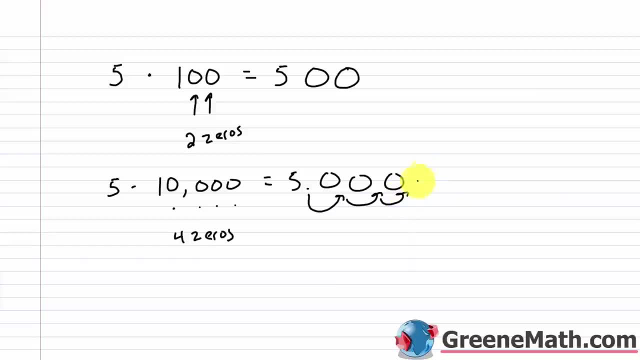 this decimal point 1, 2, 3, 4 places to the right, and I would end up with 50,000. Right? So 5 times 10,000 is 50,000. I could keep doing this. Let's do one more. Let's say we had 5 times 1 million. 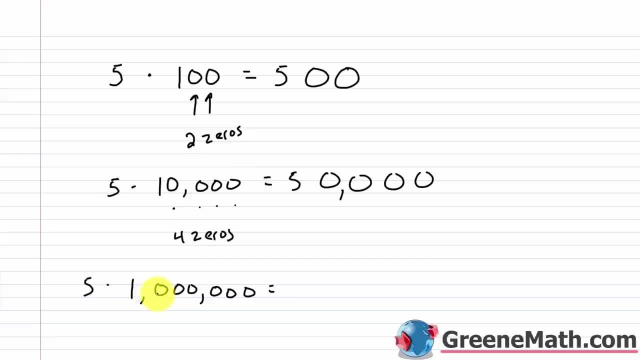 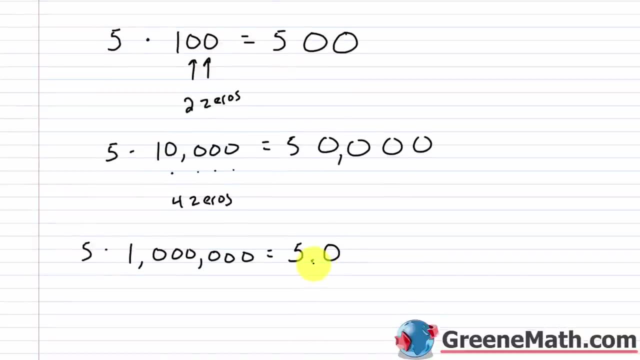 So we have 1, 2, 3, 4, 5, 6 zeros. So I could put a 5 here, 0.0. And I'm going to move this 6 places to the right. So let me go ahead and add 1, 2, 3, 4, 5 zeros. So this can go 1, 2, 3, 4, 5, 6 places to the right. And I'm going to end up with the number 5 million. All right. So additionally, I want you to recall that we have a shortcut to a zero. So we're going to go ahead and add 1, 2, 3, 4, 5, 6 zeros. So I'm going to go ahead and add 1, 2, 3, 4, 5, 6 zeros. And I'm going to 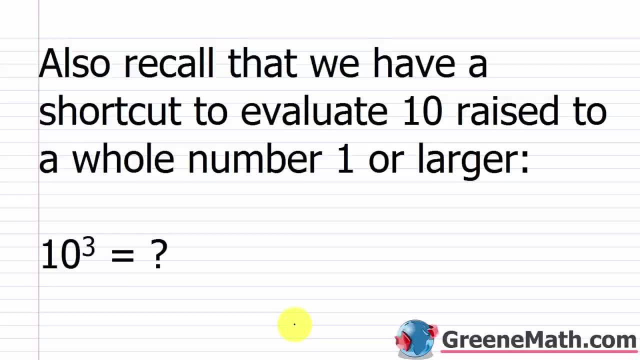 10 raised to a whole number that's 1 or larger. So 10 cubed is what? It's a 1 followed by three zeros. 1, 2, 3. So if I multiply by 10 cubed, or if I multiply by 1,000, I'm moving the decimal point three places to the right because I have 1, 2, 3 zeros there. Right? So the exponent is 3. 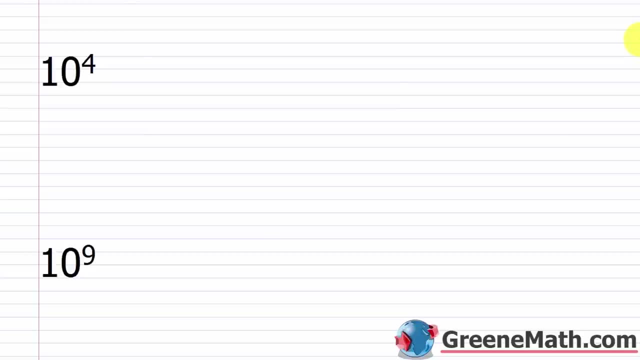 That gives me the number of zeros in that power of 10. So 10 to the fourth, that's a 1 followed by 1, 2, 3, 4 zeros. 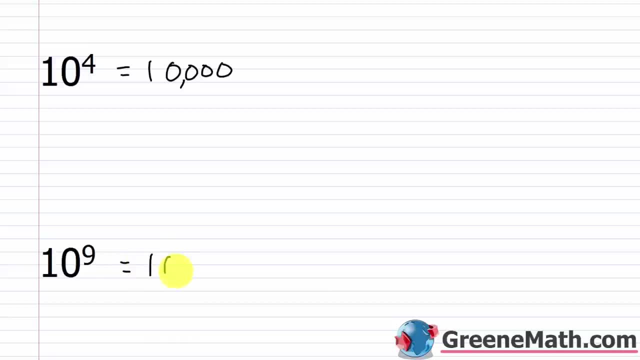 That's 10,000. 10 to the ninth is a 1 followed by 1, 2, 3, 4, 5, 6, 7, 8, 9 zeros. 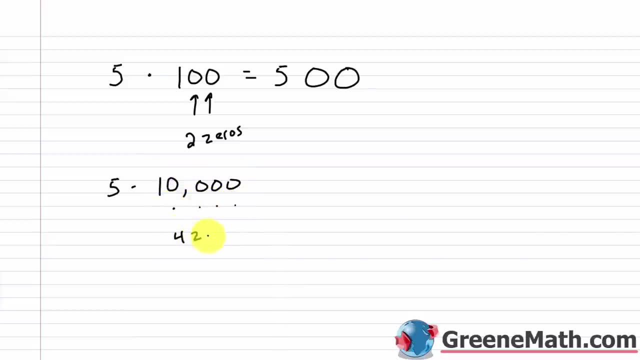 So there's one, two, three, four zeros, So four zeros. So again I could put equals five point zero And I can move this decimal point one place to the right for every zero in this power of 10.. So I can move this decimal point one, two, three, four places to the right and I would end up with 50,000, right. 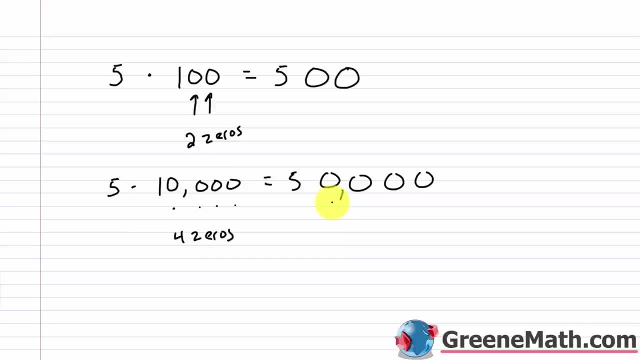 So five times 10,000 is 50,000.. I could keep doing this. Let's do one more. Let's say we had five times one million, So we have one, two, three, four, five, six zeros. 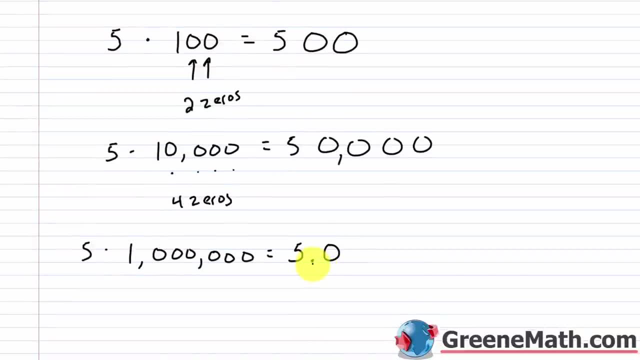 So I could put a five here, point zero, and I'm going to move this six places to the right, So let me go ahead. I'm going to add one, two, three, four, five zeros, So this can go one, two, three, four, five, six places to the right. 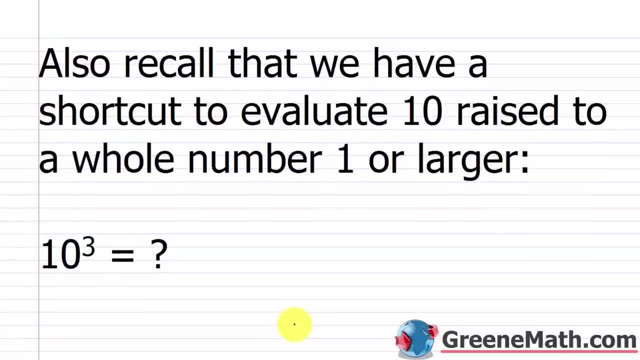 And I'm going to end up with the number: five million, All right. So, additionally, I want you to recall that we have a shortcut to evaluate: 10 raised to a whole number that's one or larger. So 10 cubed is what. 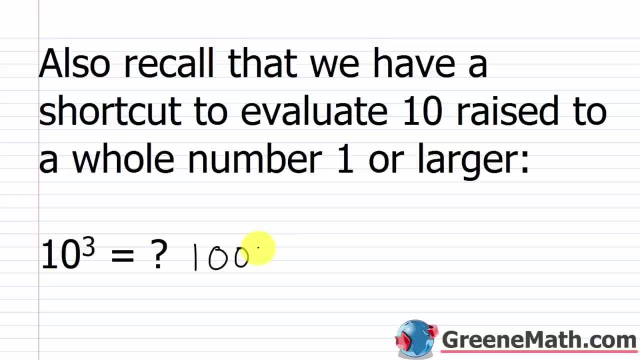 It's a one followed by three zeros: One, two, three. So if I multiply by 10, cubed, Or if I multiply by a thousand, I'm moving the decimal point three places to the right, because I have one, two, three zeros there, right. 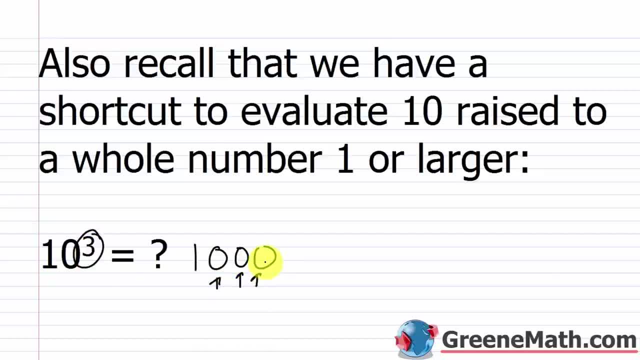 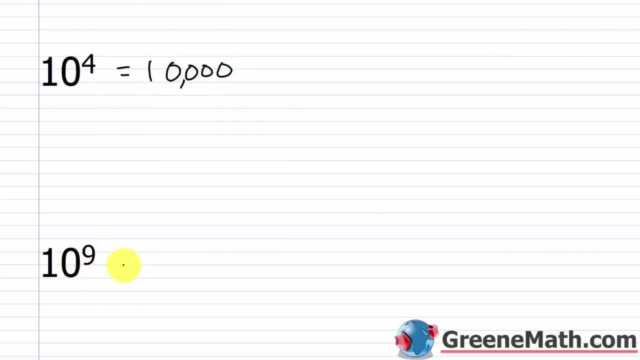 So the exponent is three. That gives me the number of zeros in that power of 10.. So 10 to the fourth, that's a one, followed by one, two, three, four zeros. That's 10,000.. 10 to the ninth is a one followed by one, two, three, four, five, six, seven, eight, nine zeros. 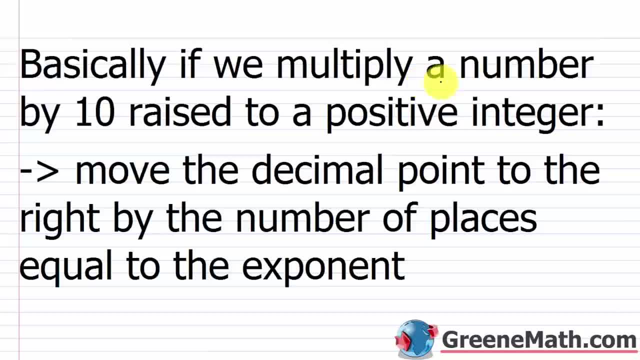 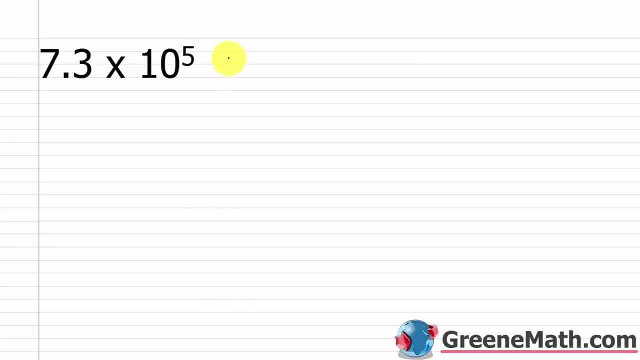 So that is one billion. So I have here. basically, if we multiply a number by 10, raised to a positive integer, we move the decimal point to the right by the number of places equal to the exponent. So, for example, if we have 7.3 times 10 to the fifth power, this number right here I can just copy it: 7.3.. 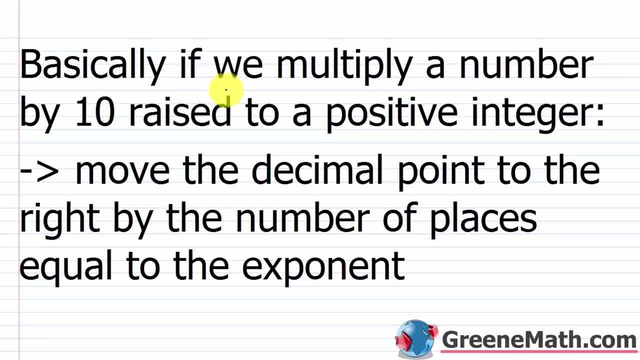 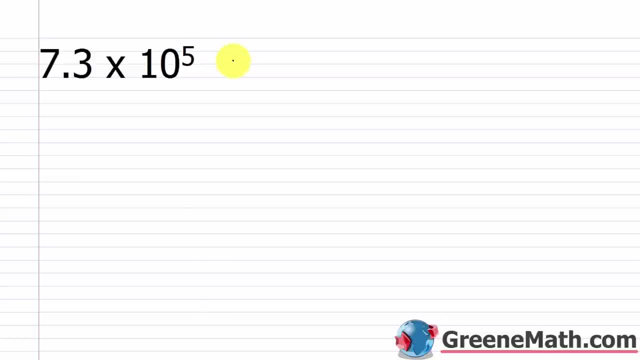 So that is 1 billion. So I have here, basically, if we multiply a number by 10 raised to a positive integer, we move the decimal point to the right by the number of places equal to the exponent. So for example, if we have 7.3 times 10 to the fifth power, this number right here, I can just come up with a number of zeros. So I'm going to go ahead and add 1 to the fifth copy at 7.3. I'm multiplying by 10 to the fifth power. So I'm multiplying by a power of 10 with what? Five zeros. So the decimal point just goes five places to the right. So let me go ahead and add four zeros behind that three. And I'm going to go 1, 2, 3, 4, 5 places to the right. And my decimal point would be there. So I'd end up with 730,000. About 6.829 times 10 to the fourth. 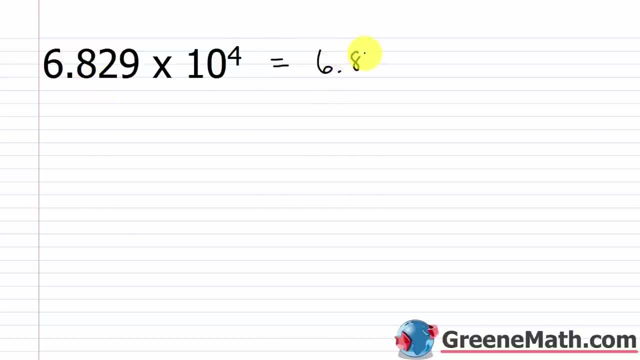 Again, just copy this number right here, 6.829. And I'm multiplying by 10 to the fourth. So the exponent is 4. If I was to evaluate 10 to the fourth power, it'd be a 1 followed by four zeros. That power of 10 would tell me to move this decimal point four places to the right if I'm multiplying by that. So this would go 1, 2, 3, put a zero behind that 9, four places to the right. And so I'd end up with 68,290. So additionally, we have a similar 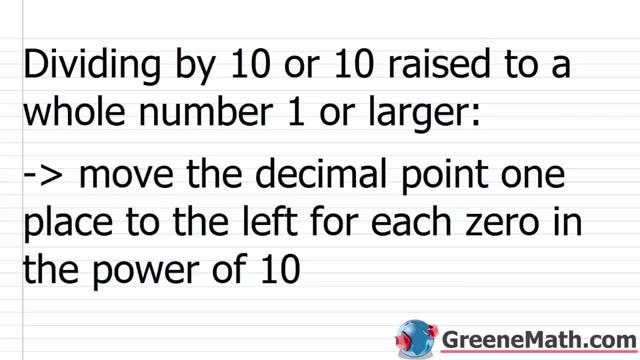 when dividing by 10 or a positive integer power of 10. So dividing by 10 or a 10 raised to a whole number one or larger. So we're going to move the decimal point one place to the left for each zero and the power of 10. Now, if I'm multiplying by 10 or a 10 raised to a whole number one or larger, I'm just moving the decimal point one place to the right for each zero and the power of 10. So 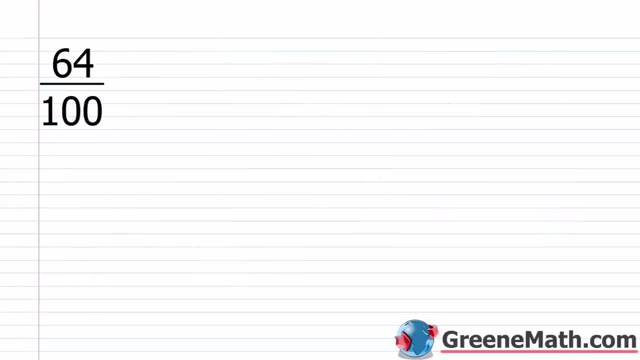 it's left for division, right for multiplication. So for example, I have 64 divided by 100. 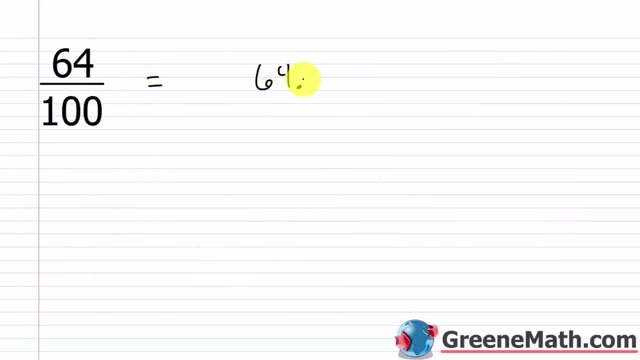 I'll take 64, put a visible decimal point here. I've got two zeros. So this is going to go one, two places to the left, and I'll end up with 0.64, or a lot of people would like to write 0.64. 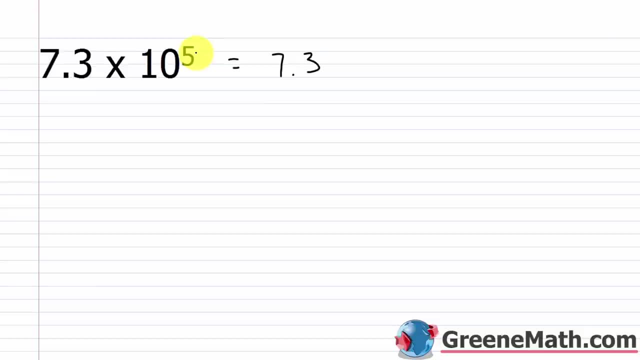 I'm multiplying by 10 to the fifth power. So I'm multiplying by a power of 10. with what? Five zeros? So the decimal point just goes five places to the right. So let me go ahead and add four zeros behind that three. 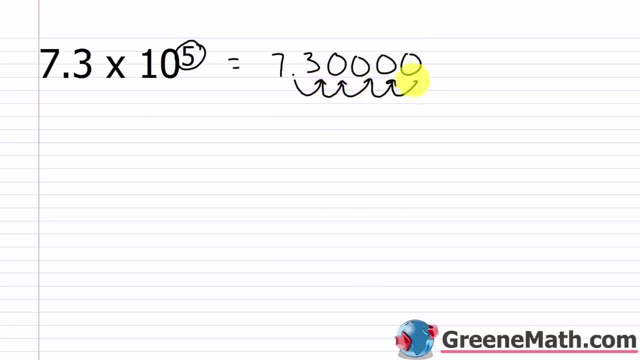 And I'm going to go one, two, three, four, five places to the right And my decimal point would be there, So I'd end up with 730,000.. About 6.829 times 10. to the fourth. 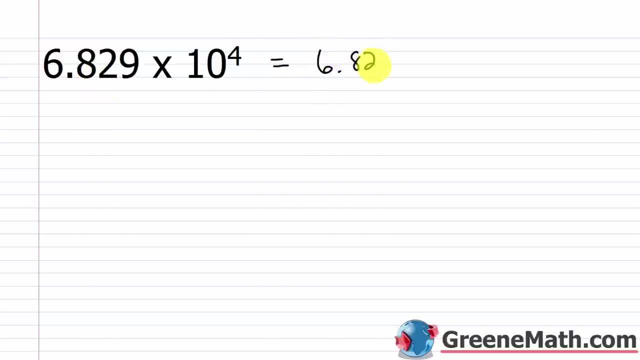 Again. just copy this number right here: 6.829.. And I'm multiplying by 10 to the fourth, So the exponent is four. If I was to evaluate 10 to the fourth power, it'd be a one followed by four zeros. 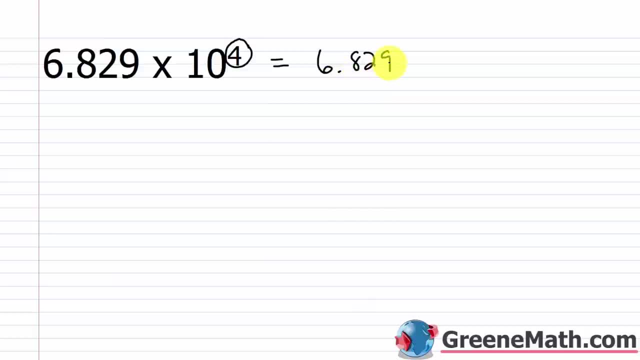 That power of 10 would tell me to move this decimal point four places to the right, if I'm multiplying by that. So this would go one, two, three, put a zero behind that nine, four places to the right, And so I'd end up with 68,290. 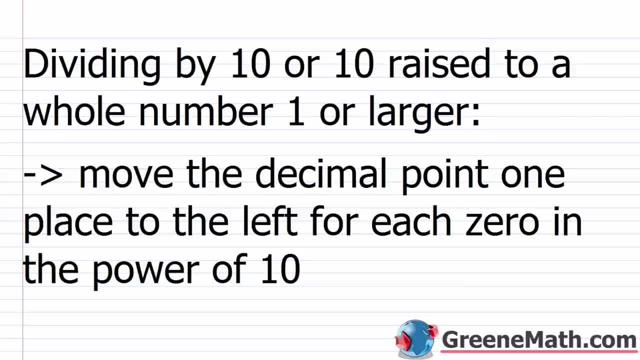 So, additionally, we have a similar trick when dividing by 10, or a positive integer power of 10.. So dividing by 10, or a 10, raised to a whole number, one or larger. So we're going to move the decimal point one place to the right. 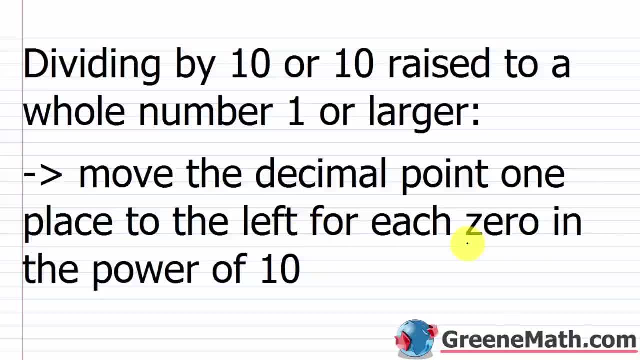 So we're going to move the decimal point one place to the left. So we're going to move the decimal point one place to the left for each zero and the power of 10.. Now, if I'm multiplying by 10 or a 10 raised to a whole number, one or larger. 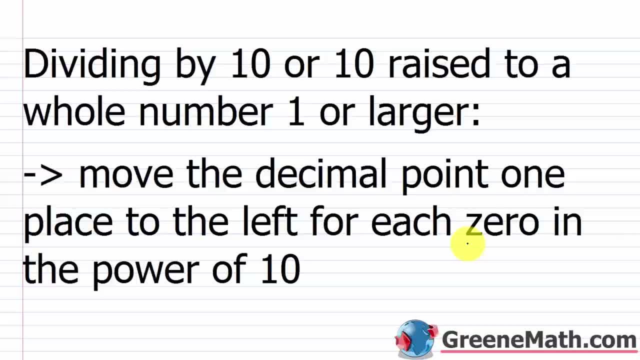 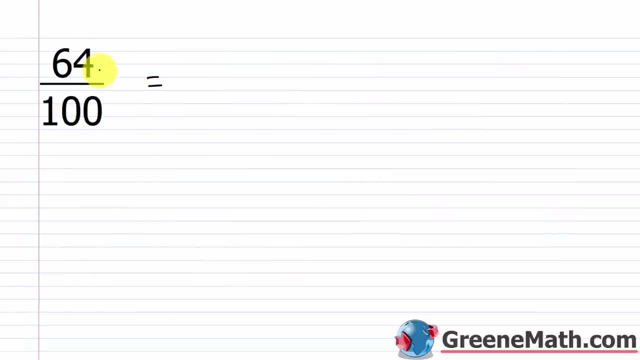 I'm just moving the decimal point one place to the right for each zero and the power of 10.. So it's left for division, right for multiplication. So for example, I have 64 divided by 100.. I'll take 64, put a visible decimal point here. 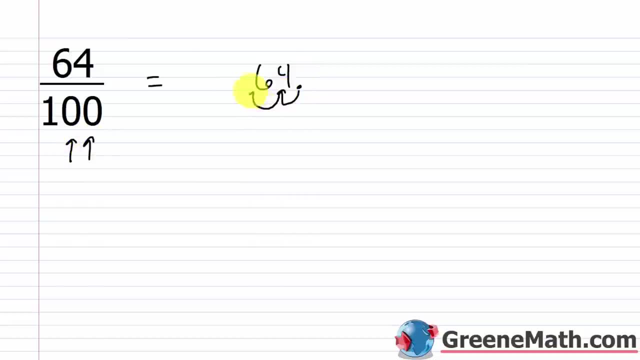 I've got two zeros, So this is going to go one, two places to the left And I'll end up with 0.64.. Or a lot of people will say, oh, that's not right, But a lot of people would like to write 0.64. 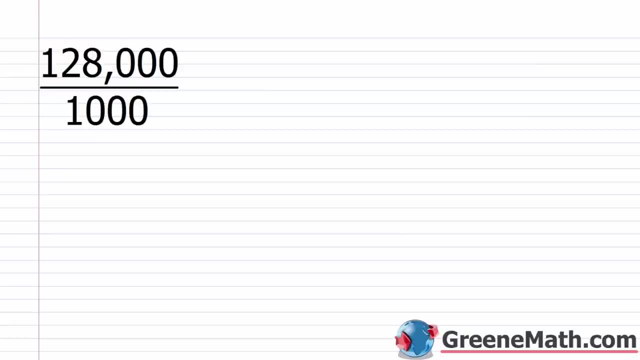 What about 128,000 over 1,000?? One trick is to cancel zeros. So in other words, I can take this and cancel with this. Every time I'm doing that, I'm removing a factor of 10.. So I'm canceling this with this, this with this. 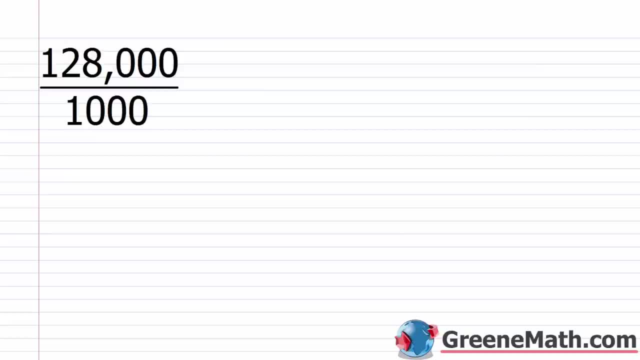 What about 128,000 over 1,000? One trick is to cancel zeros. So in other words, I can take this and cancel with this. Every time I'm doing that, I'm removing a factor of 10. So I'm canceling this with this, this with this, and I'll end up with 128 over 1. But another way I could have done that, another way I could have done that is just writing 128,000. Put my decimal 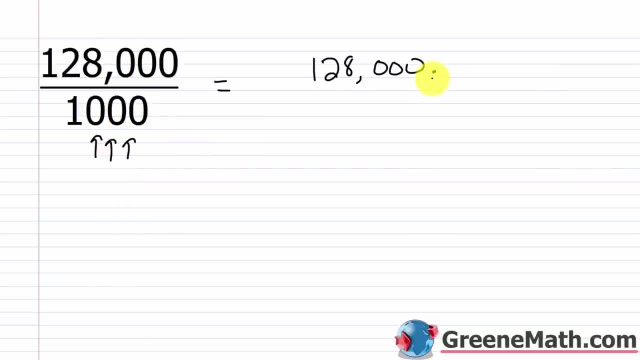 point here. I've got one, two, three zeros. So I would move this one, two, three places to the left. 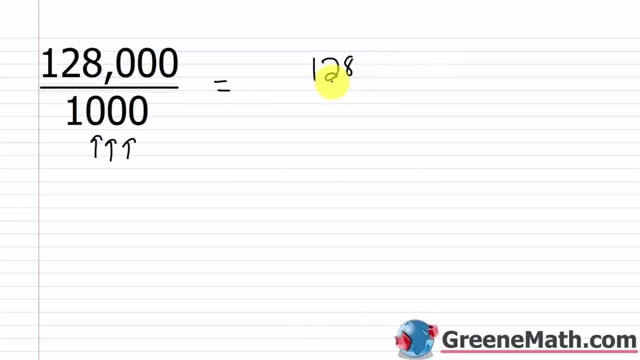 And again, I'd end up with the number 128 either way. What about 64 times 10 to the power of 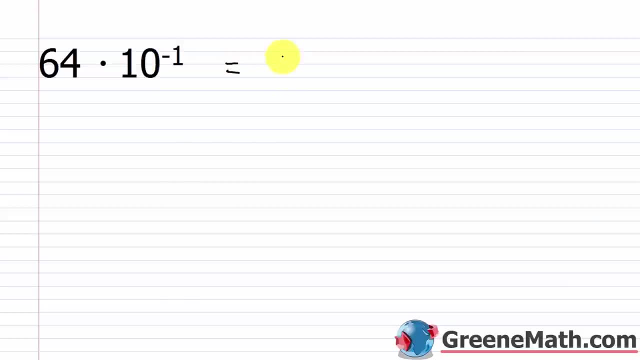 negative one? We learned about negative exponents in our last lesson. So this would be 64 times 10 to the power 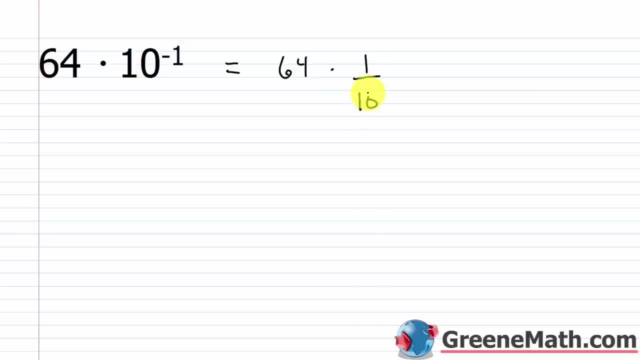 of negative one is one-tenth, right? It's one over 10 to the power of one, so one-tenth. And so essentially here, you have 64 divided by 10. And so I can do this as saying, okay, I have 64, 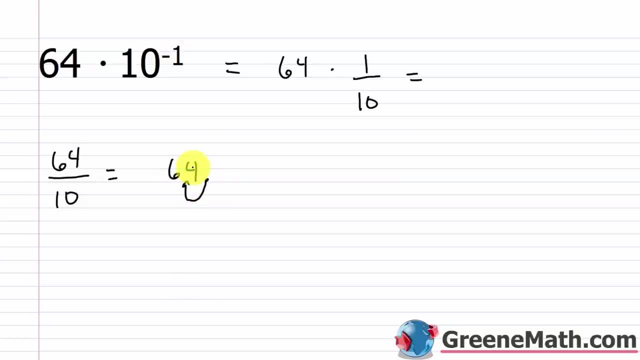 put the decimal point at the end, and then move this one place to the left, 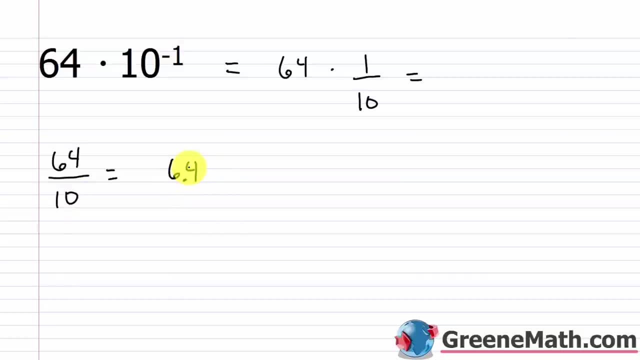 because I have one zero here. So this would end up being 6.4. So let's revisit a problem real quick. So I'm going to take 128,000 times 10 to the power of negative 3. We've done this a few 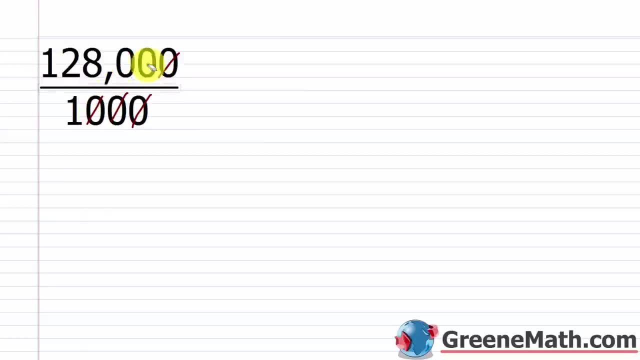 And I'll end up with 128 over 1.. But another way I could have done that. another way I could have done that is just writing 128,000.. Put my decimal point here. I've got one, two, three zeros. 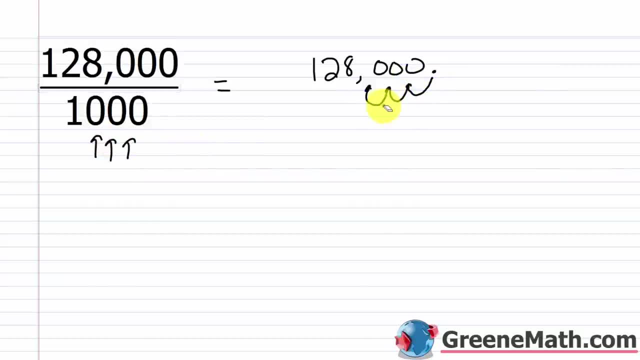 So I would move this one, two, three places to the left, And again I'd end up with the number 128. either way, What about 64 times 10 to the power of negative 1?? We learned about negative exponents in our last lesson. 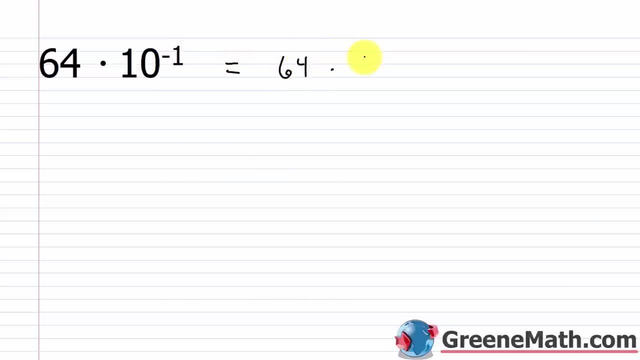 So this would be 64 times 10 to the power of negative. 1 is 1 tenth. Right, it's 1 over 10 to the power of 1.. So 1 tenth. And so essentially here we're going to have 1 over 10 to the power of 1.. 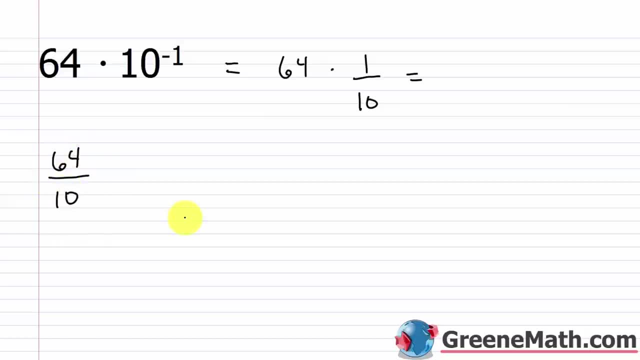 And here you have 64 divided by 10.. And so I can do this as saying: okay, I have 64.. Put the decimal point at the end And then move this one place to the left, because I have one zero here. 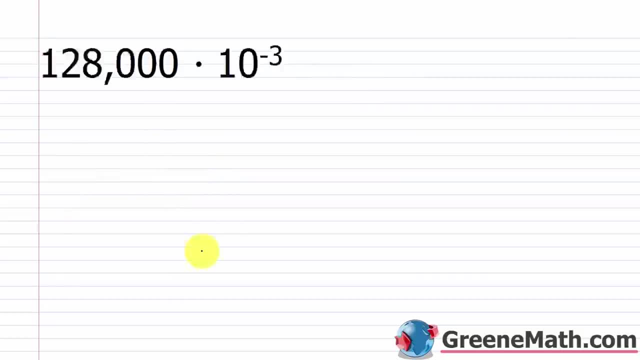 So this would end up being 6.4.. So let's revisit a problem real quickly. We have 128,000 times 10 to the power of negative 3.. We've done this a few examples ago, but it just looked different. 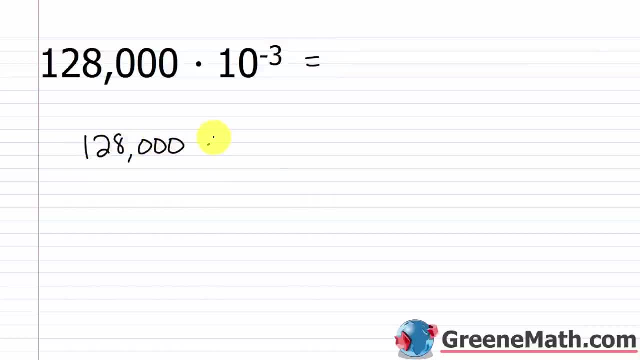 We have 128,000 times 10 to the power of negative 3 is 1 over 10 to the power of negative 3.. We have 128,000 over 10 cubed, or 1 over 1,000, right. 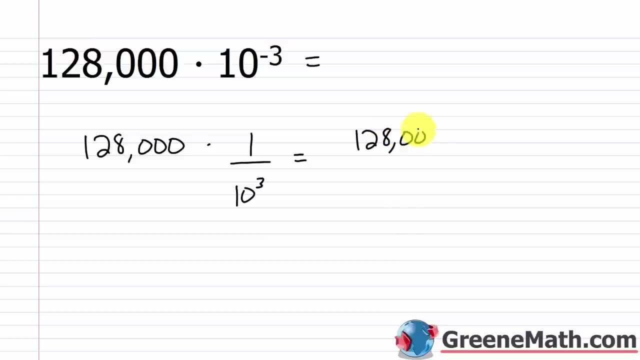 So I can really write this as 128,000 over 1,000 or 10 cubed. So really, again, I'm taking 128,000 and I'm taking my decimal point. I'm moving it three places to the left. 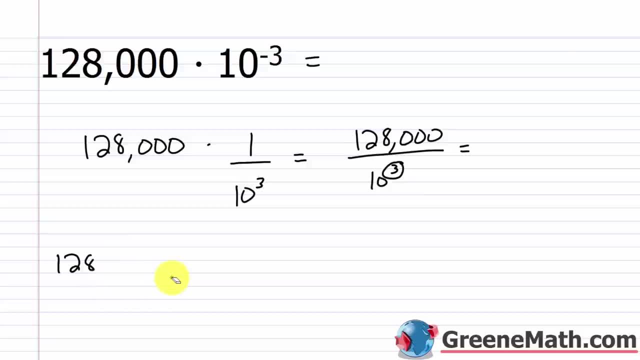 1, 2, 3.. That's going to give me the number 128.. So for the next one, I have 5.476 times 10 to the power of negative 4.. So do I need to keep writing this as 5.476 times 1 over 10 to the fourth power? 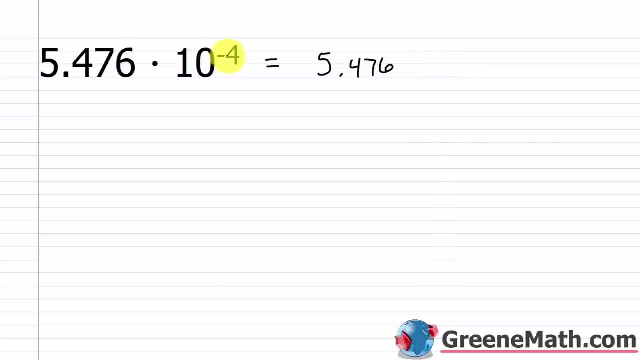 I don't, Because what I need to realize here is that I'm just going to take, if I have a negative exponent on 10, okay, something like negative 4, all that's going to end up happening is I'm going to take this value here. 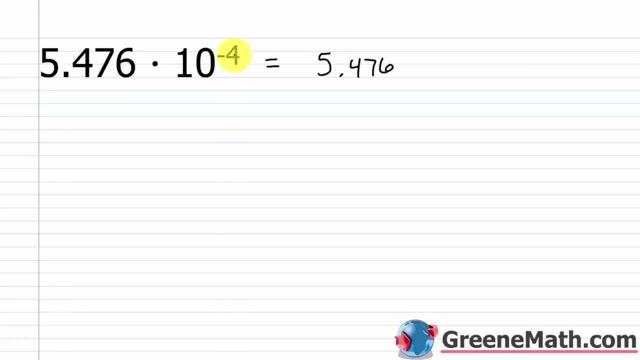 and I'm going to move my decimal point four places to the left right If it's a negative 4.. If it was a negative 7, I'd move it seven places to the left. If it was a negative 12, I'd go 12 places to the left. 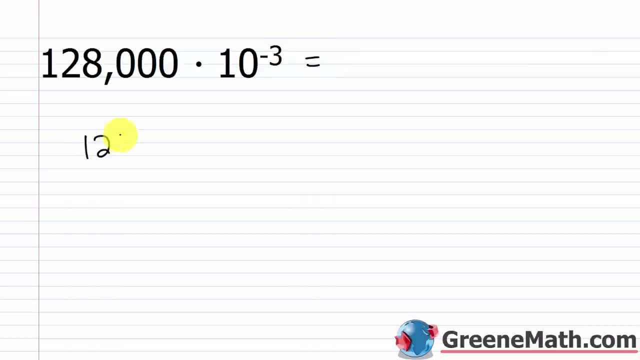 examples ago, but it just looked different. We have 128,000 times 10 to the power of negative 3 is one over 10 cubed, or one over 1,000, right? So I could really write this as 128,000 over 1,000, or 10 cubed. So really, again, I'm taking 128,000, and I'm taking my decimal point, and I'm moving it three places to the left. One, two, three. That's going to give me the number 128. So for the next one, I have 5.476 times 10 to the power of negative 4. So do I need to keep writing this as 5.476 times 1 over 10 to the fourth power? I don't. Because what I need to realize here is that I'm just going to take, if I have a negative exponent on 10, okay, something like negative 4, all that's going to end up happening is I'm going to take this, this value here, and I'm going to move my decimal point four places to the left, right? If it's a negative 4. If it was a negative 7, I'd move it seven places to the left. If it was a negative 12, I'd go 12 places to the left. So really, all I need to do is write this number, 5.476, and then look at that and say, okay, it's a negative. So that means I'm going to go to the left, and then by four places, right? Because the exponent is negative 4. So this would go 1, 2, 4 places to the left, right there. You'd have 0.0005476 as your answer. And if you wanted to, you could do that the long way. You could have written this as 5.476 times 1 over 10 to the 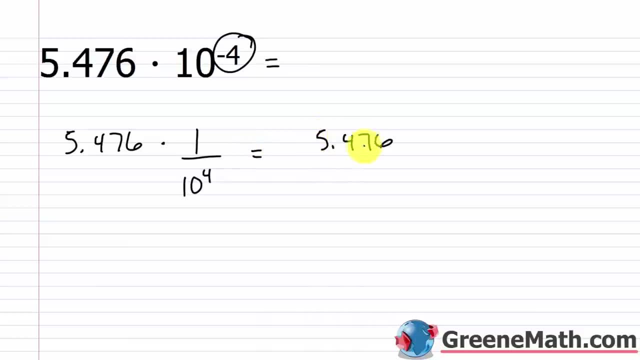 fourth power. I said, okay, I have 5.476 over 10 to the fourth power. I said, okay, well, I have four zeros in this power of 10 that I'm dividing by. So yeah, this is going to be 5.476. This is going to move 1, 2, 3, 4 places to the left. 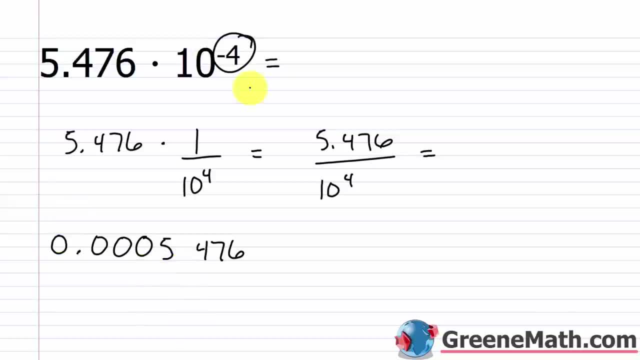 But again, the way I showed you a minute ago was much, much quicker. I don't have all this tedious stuff I've got to go through. All right, now that we've reviewed everything, let's talk a little bit 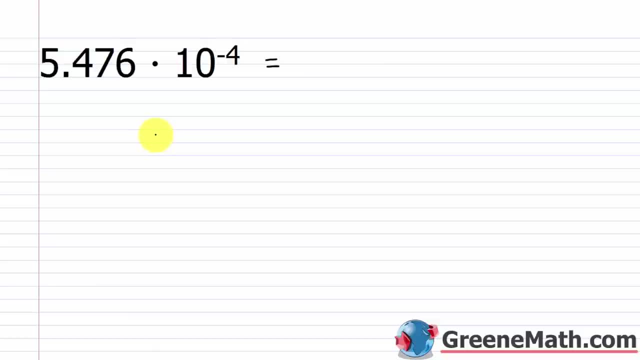 So Really all I need to do is write this number- 5.476, and then look at that and say, okay, it's a negative. So that means I'm going to go to the left, and then by four places, right? 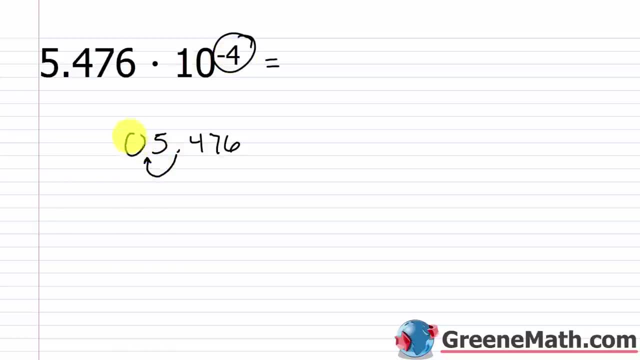 Because the exponent is negative 4.. So this would go 1,, 2,, 3,, 4 places to the left, Right. there You'd have 0.0005476 as your answer, And if you wanted to, you could do that. 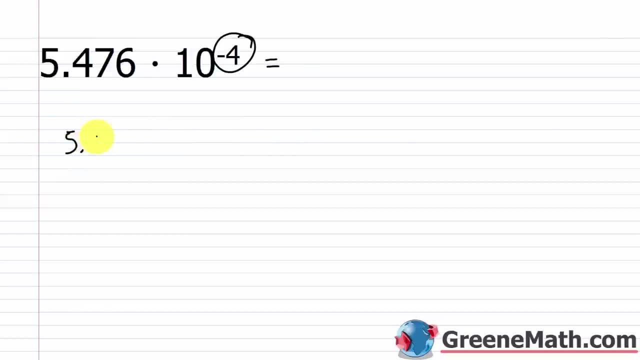 The long way you could have written this as: 5.476 times 1 over 10 to the fourth power. said okay, I'll have 5.476 over 10 to the fourth power and said, okay, well, I have four zeros in this power of 10 that I'm dividing by. 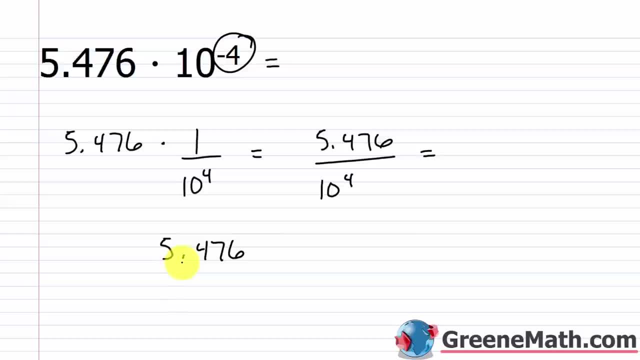 So yeah, this is going to be 5.476.. This is going to move 1,, 2,, 3, 4 places to the left, But again, the way I showed you a minute ago, it was much, much quicker. 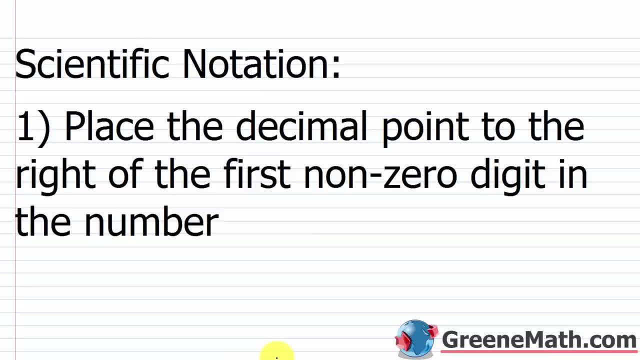 I don't have all this tedious stuff I've got to go through All right. Now that we've reviewed everything, let's talk a little bit about scientific notation. So it's kind of easy to do this. The first thing you want to do is place the decimal point to the right. 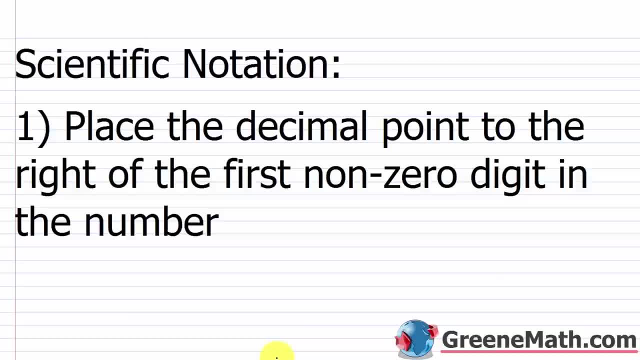 of the first non-zero digit number. So if the number was, let's say, 672,, the first non-zero digit means coming from the left and going to the right. This is non-zero, So it's going to the right of that first digit. 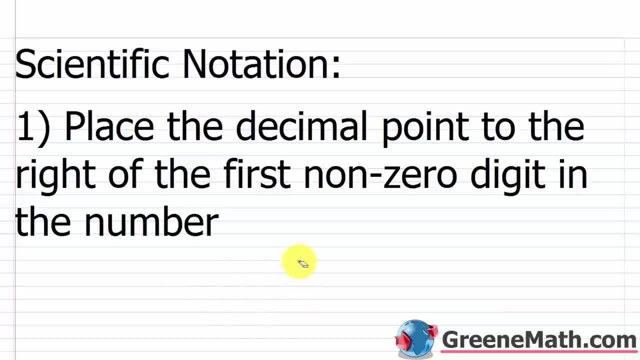 So that's where my decimal point is going to go. If I had something with with a bunch of zeros- let's say I had .00000027506,, this is going to get moved to right there. Ignore the zeros. You're coming from the left and going to the right. 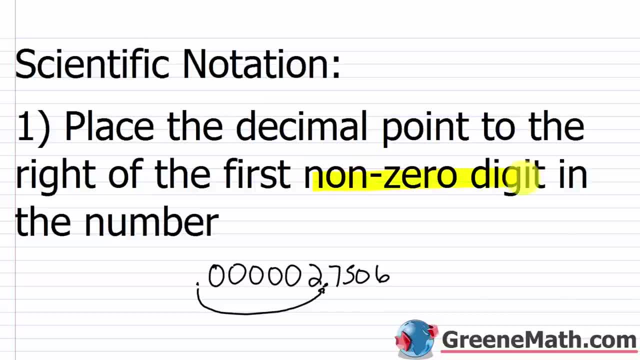 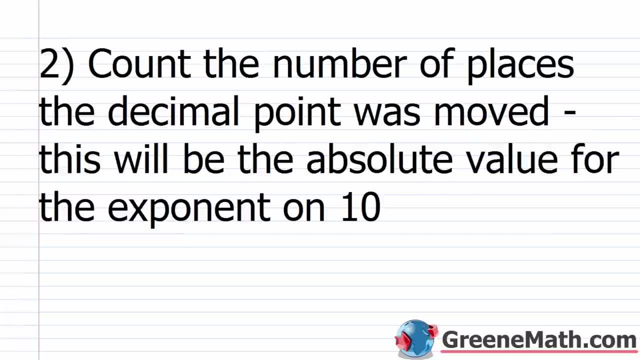 So it's to the right of the first non-zero digit. It's got to go right there, Okay, So that's kind of your first step with scientific notation. Now the second thing you're going to do is count the number of places the decimal point was moved. 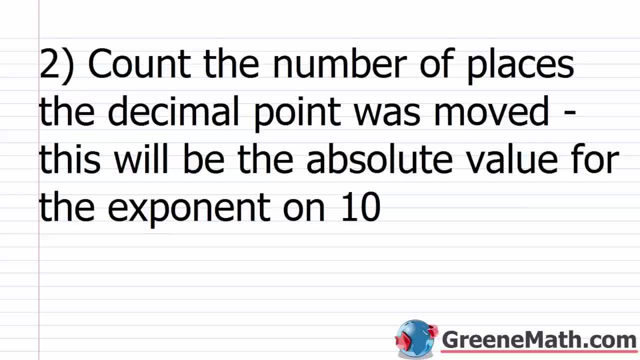 This will be the absolute value for the exponent on 10.. So again count the number of places. you moved that decimal point. So let's say I had something like 682.. Well, my decimal point is here and I'm going to move it here, right? 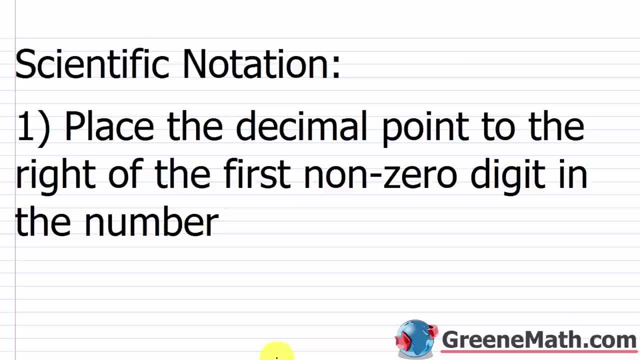 about scientific notation. So it's kind of easy to do this. The first thing you want to do is place the decimal point to the right of the first non-zero digit number. So if the number was, 2, the first non-zero digit means coming from the left and going to the right. This is non-zero, so it's going to the right of that first digit. So that's where my decimal point's going to go. 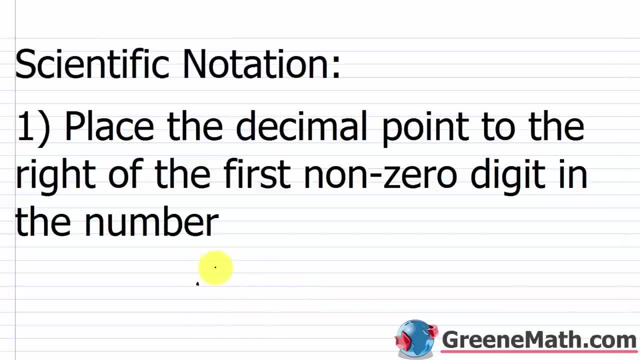 If I had something with a bunch of zeros, let's say I had 0.000027506, this is going to get moved to right there. Ignore the zeros. You're coming from the left and going to the right. So it's to the right of the first non-zero digit. So if I had something with a bunch of zeros, let's say I had 0.000027506, this is going to get moved to right there. So that's kind of your first step 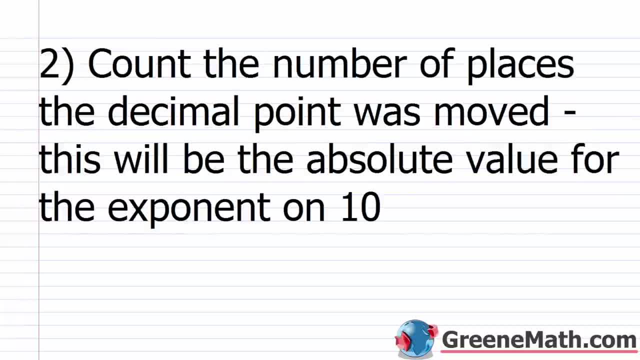 with scientific notation. Now, the second thing you're going to do is count the number of places the decimal point was moved. This will be the absolute value for the exponent on 10. So again, 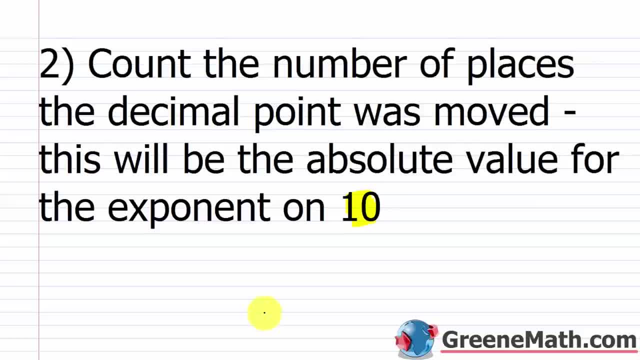 count the number of places you moved that decimal point. So let's say I had something like 682. Well, my decimal point is here, and I'm going to move it here. Because I'm moving it immediately after the first non-zero digit. So it's going to go there. 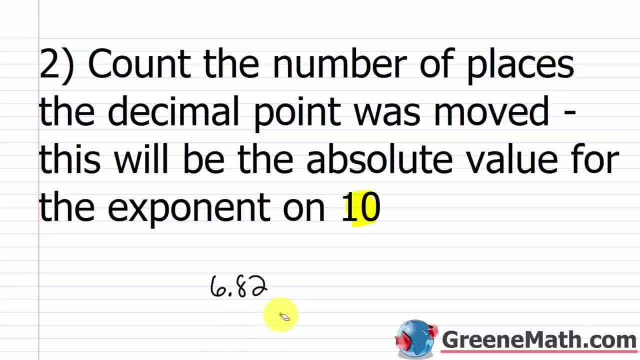 So it went one, two places to the left. So I'm going to say, okay, the number that I'm looking for is a two. That's going to be the absolute value for the exponent on 10. Or something like 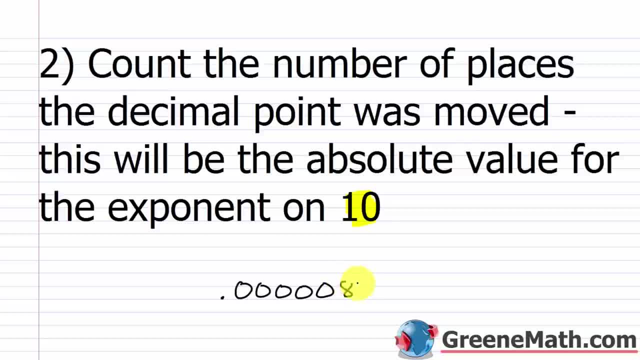 0.000000812. This is going to go here. I'm going to move it one, two, three, four, five, six places to the right. So the absolute value for the exponent on 10 is going to go here. 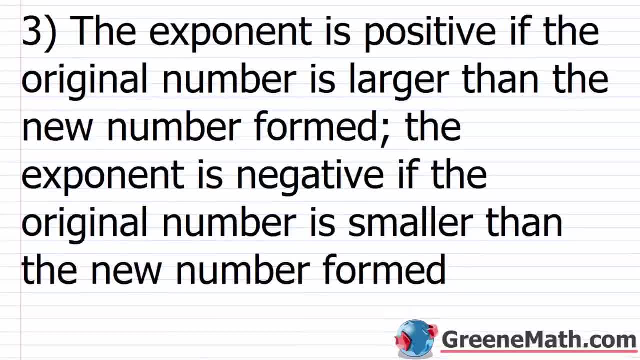 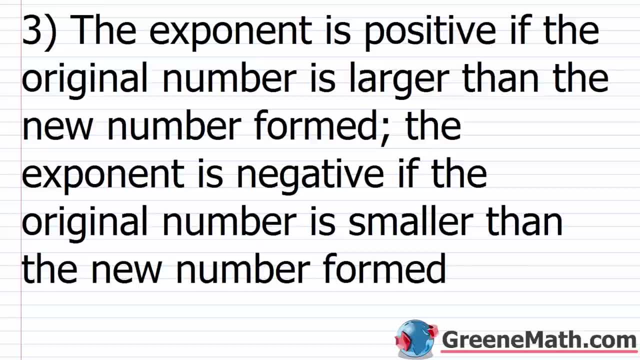 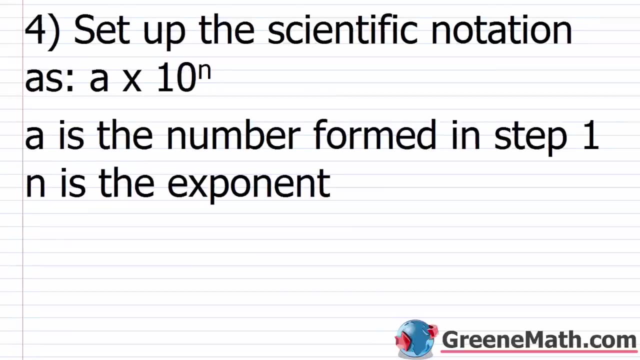 The exponent on 10 will be a six in this case. Now, step three. The exponent is positive if the original number is larger than the new number formed. Then the exponent is negative if the original number is smaller than the new number formed. And that's going to make sense once we start doing some examples. And then for step four, we just set up the scientific notation 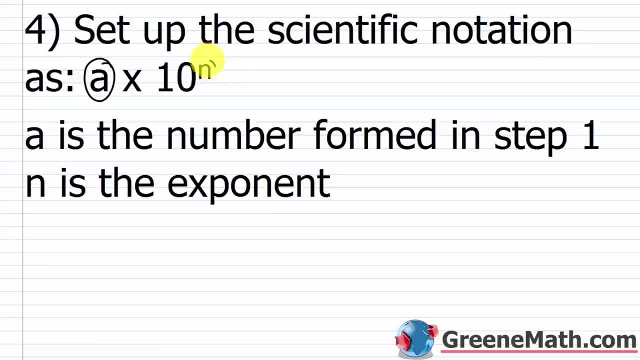 as a times 10 to the power of n. 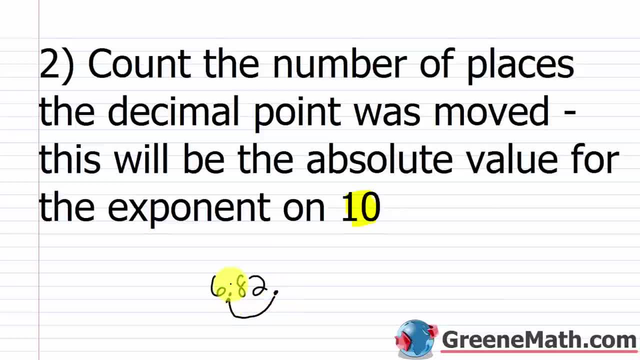 because I'm moving it immediately after the first non-zero digit. So it's going to go there. So it went one, two places to the left. So I'm going to say, okay, the number that I'm looking for is a 2.. 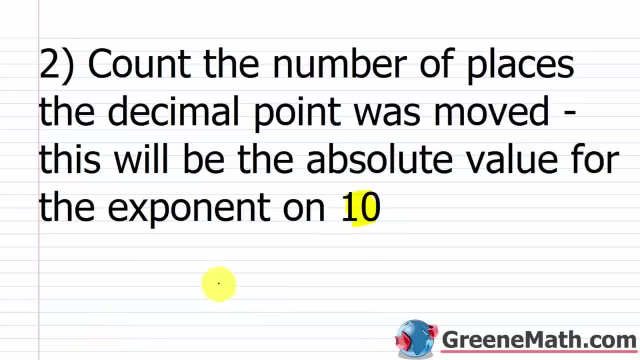 That's going to be the absolute value for the exponent on 10.. Or something like .000000812.. This is going to go here. I'm going to move it one, two, three, four, five, six places to the right. 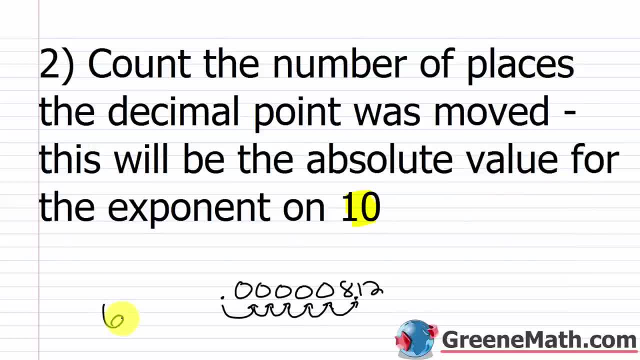 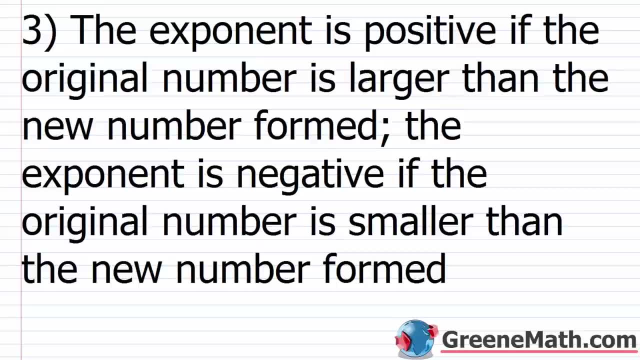 So the absolute value for the exponent on 10 will be a 6 in this case. Now step three. the exponent is positive if the original number is larger than the new number formed. Then the exponent is positive if the original number is larger than the new number formed. 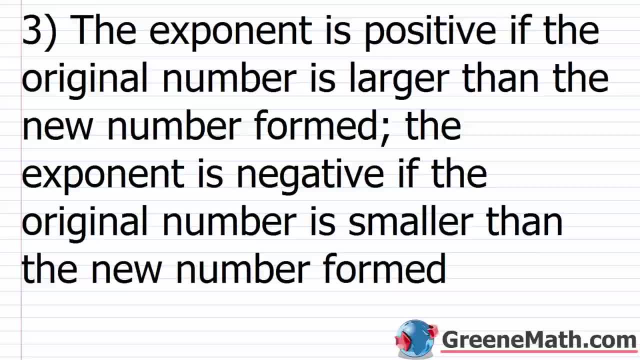 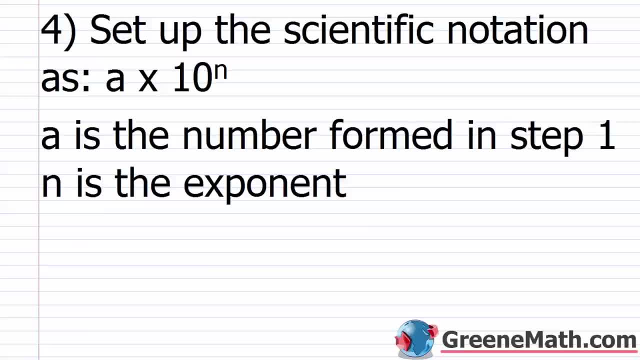 Then the exponent is negative if the original number is smaller than the new number formed. And that's going to make sense once we start doing some examples. And then, for step four, we just set up the scientific notation as a times 10 to the power. 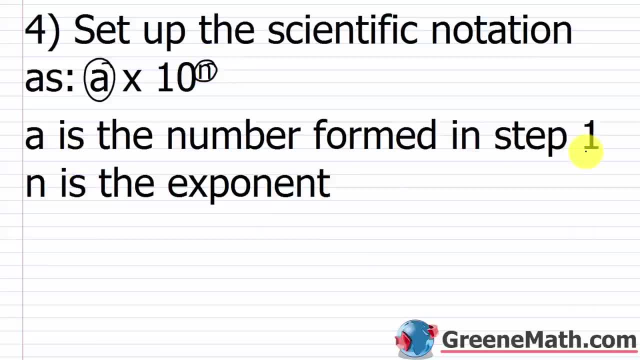 of n, where a is the number formed in step one right, where we had put a decimal point after the first non-zero digit. Then n is going to be the exponent. We got that in step two right. We counted the number of places. 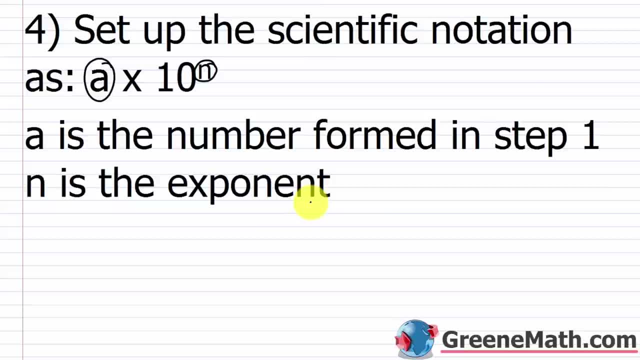 We counted the number of places that we had to move our decimal point And in step three we figured out what the sign was going to be. Now, I know these steps. when you kind of just read them out loud and you don't really have an example, it seems like man, it's going to be really difficult. 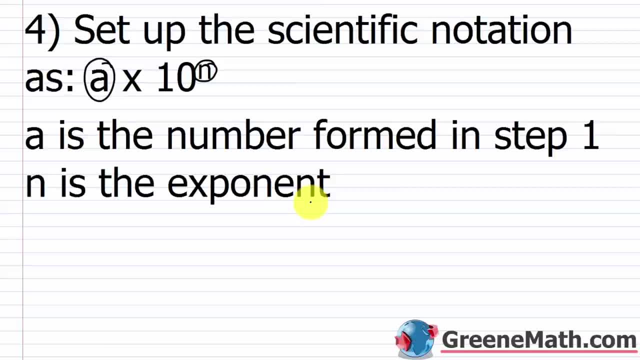 You practice 10 or 15 of these, you're going to really have this down pat. It's super, super easy. All right, let's take a look at an example. So we have 96 million and we want to write this in scientific notation. 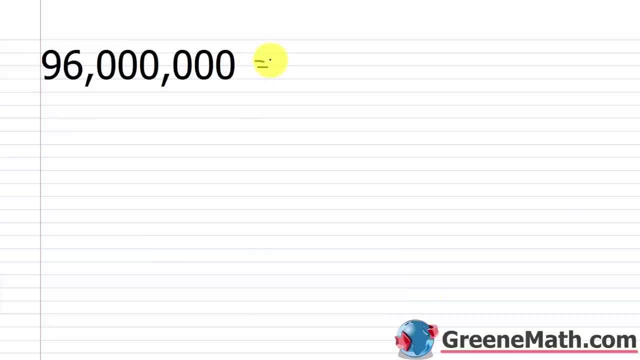 So the first thing is, again, you want to place the decimal point to the right of the first non-zero digit in the number. So, coming from the left, we're going to put the decimal point to the right of the first non-zero digit in the number. 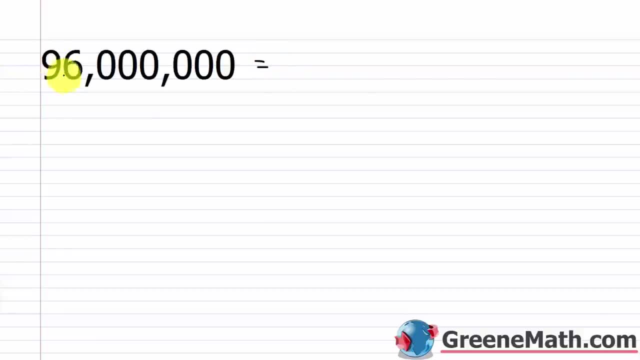 So, coming from the left, we're going to put the decimal point to the right of the first non-zero digit in the number. The first non-zero digit is a nine, so I'd put the decimal point right there, So it would be 9.6.. 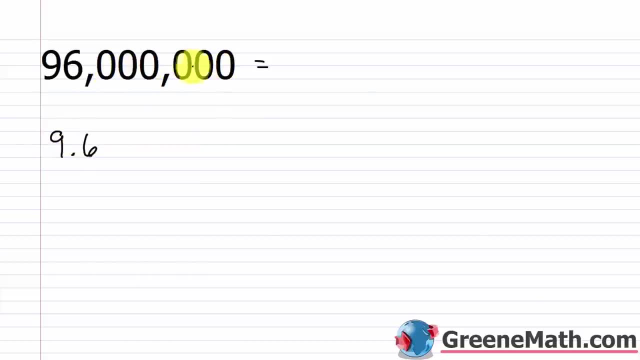 You'd have all these zeros after the six. So that's one, two, three, four, five six. So one, two, three, four, five, six. But the question is, do I want to write them? Well, they don't add any value to the number, so you don't have to. 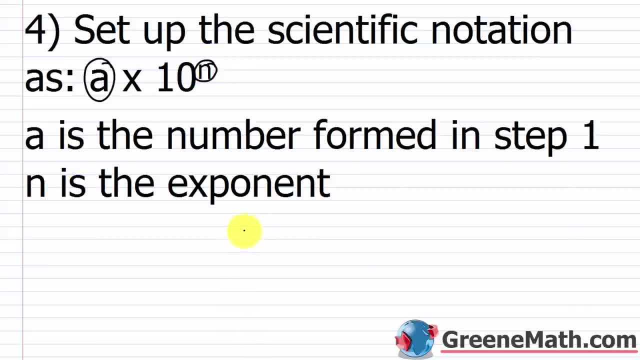 What is the number formed in step one, right? Where we had put a decimal point after the first non-zero digit. Then n is going to be the exponent. We got that in step two, right? We counted the number of places that we had to move our decimal point. And in step three, we figured out what the sign was going to be. Now, I know these steps, when you kind of just read them out loud and you don't really have an example, it seems like, man, it's going to be really difficult. You practice 10 or 15 of these, you're going to really have this down pat. It's super, super easy. All right, let's take a look at an example. 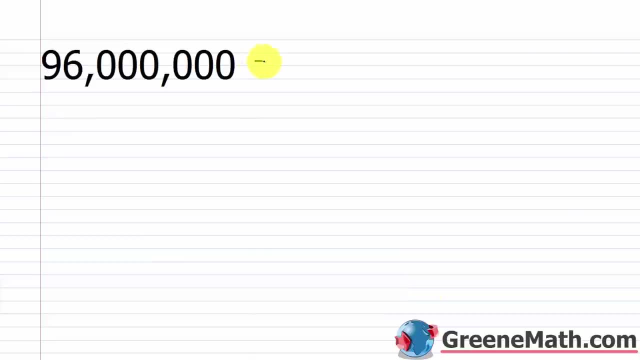 26 million. And we want to write this in scientific notation. So the first thing is, again, you want to place the decimal point to the right of the first non-zero digit in the number. 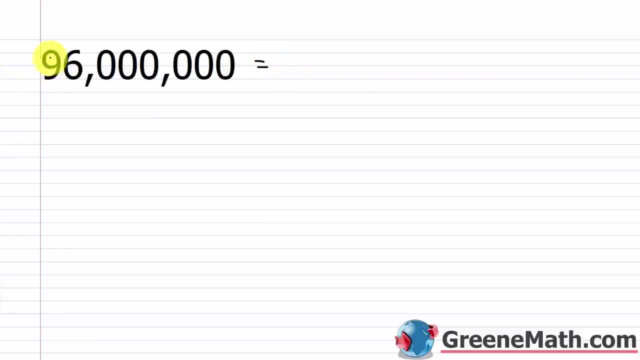 So coming from the left, going to the right, the first non-zero digit is a nine. So I'd put the decimal point right there. So it would be 9.6. You'd have all these zeros after the six. So that's 1, 2, 3, 4, 5, 6. So 1, 2, 3, 4, 5, 6. But the question is, do I want to write them? Well, they don't add any value to the number, so you don't have to. You might be asking, why don't they add any value to the number? Remember, we have a decimal point here now. So after your decimal point and the final non-zero digit, the zeros don't matter. They don't add any value. So you can just erase them. You don't need them. You just have that number 9.6. 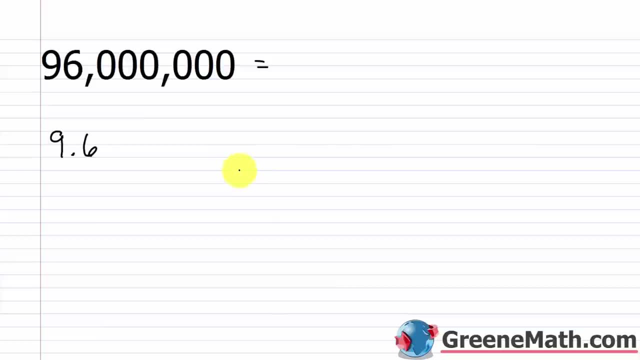 Now, these two are not equal yet, but they're going to be. Now, the next thing I want to do is count the number of places the decimal point was moved. What was moved? 1, 2, 3, 4, 5, 6, 7 places. So my exponent on 10, the absolute value of it is 7. Absolute value is 7. 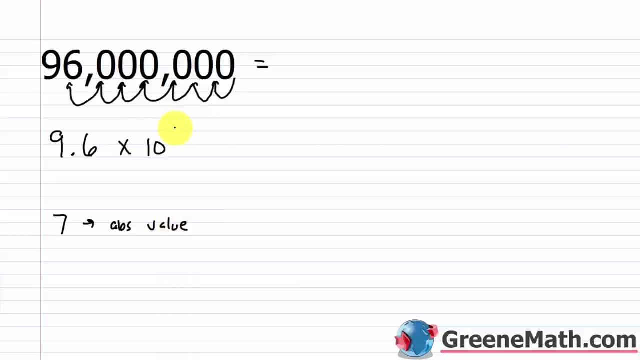 So I'm going to multiply this by 10. I know the absolute value of the exponent will be 7. But will it be positive or will it be negative, knowing the absolute value is not enough? Well, again, in step three, I told you the exponent is positive if the original number is 7. Then the new number. Here's the original number, 96 million. Here's the number that we form, 9.6. So clearly this is bigger. So the exponent would need to be positive. So this is 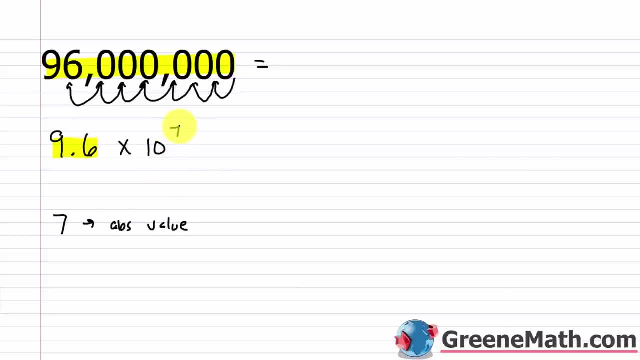 going to be positive 7. And we're done. We've written it in the form described in step four, 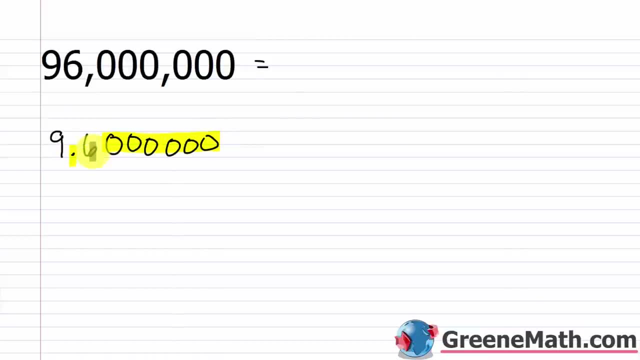 You might be asking: why don't they add any value to the number? Remember, we have a decimal point here now. So after your decimal point and the final non-zero digit, the zeros don't matter, They don't add any value, so you can just erase them. 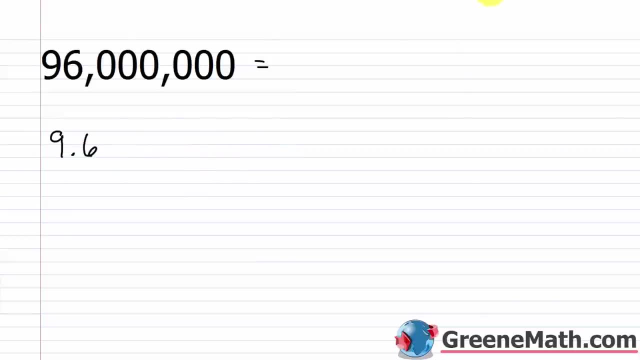 You don't need them, You just have that number, 9.6.. Now, these two are not equal yet, but they're going to be. Now, the next thing I want to do is count the number of places the decimal point was moved. 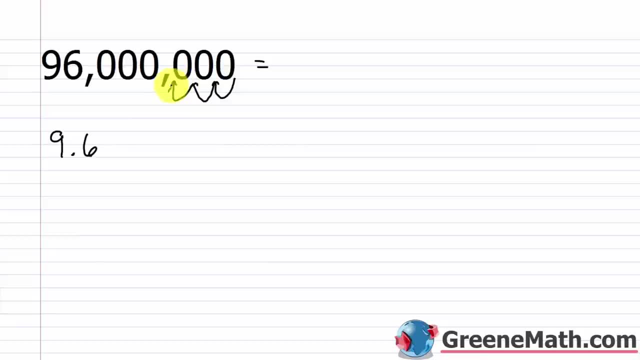 What was moved? One, two, three, four, five, six, seven places. So my exponent on 10, the absolute value of it is seven. Absolute value is seven, So I'm going to multiply this by 10.. I know the absolute value of the exponent will be seven. 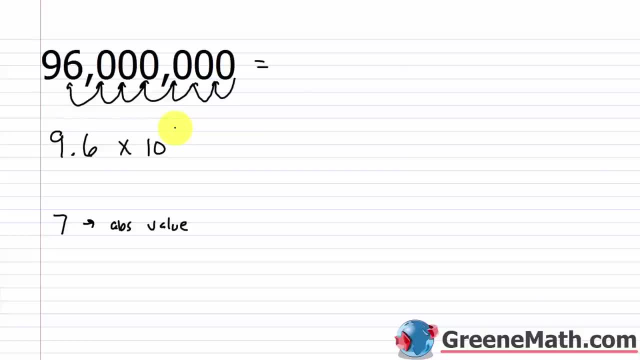 But will it be positive or will it be negative? Knowing the absolute value is not enough. Well, again, in step three, I told you the exponent is positive if the original number is larger than the new number. Here's the original number: 96 million. 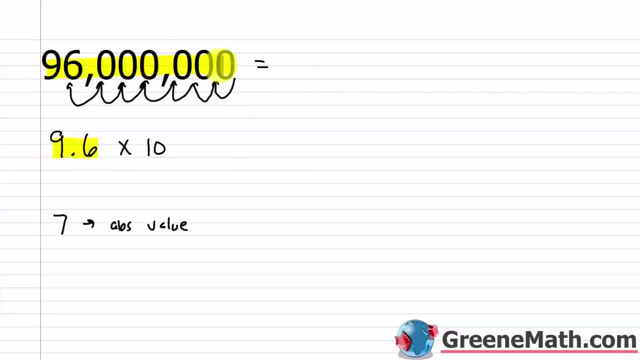 Here's the number that we form: 9.6.. So clearly this is bigger, so the exponent would need to be positive. So this is going to be positive seven and we're done. All right, we've written it in the form described in step four. 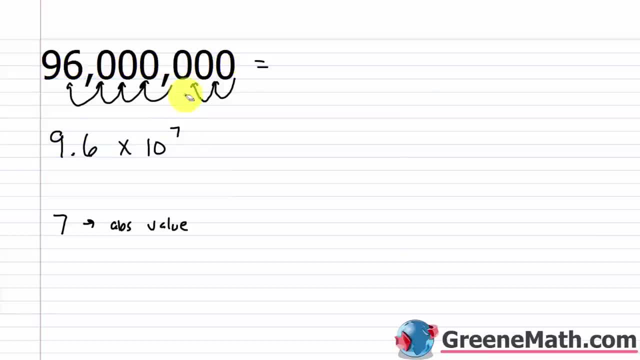 which is a times 10 to the nth power. Now a couple of pointers for you here. The first thing is that you don't need to go through this elaborate process every time To get your sign for your exponent. just think about: okay, if I'm here, 9.6,. 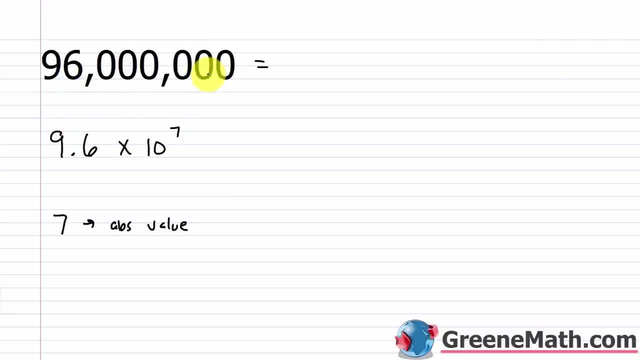 and I want to go to here- 96 million, what I need. to multiply by a power of 10. that's going to tell me to move my decimal point to the right Or the left. Remember, if this is positive, I'm going to be moving my decimal point to the right. 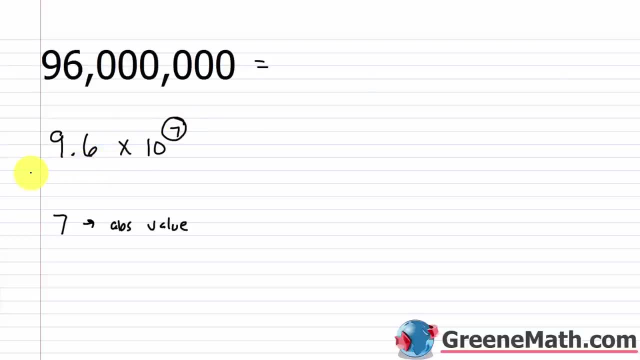 If it's negative, I'm going to be moving my decimal point to the left. I want to move this seven places to the right. I want to go one, two, three, four, five, six, seven places to the right so I can get back this original number of 96 million. 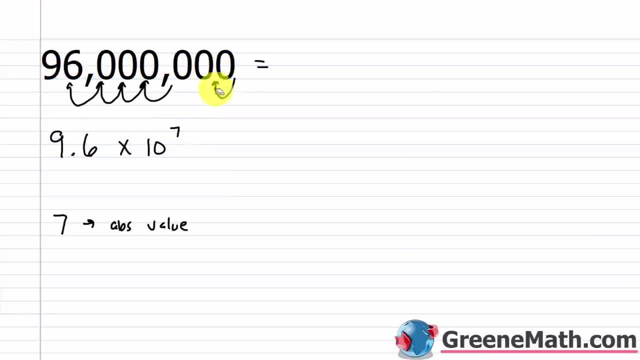 which is a times 10 to the nth power. Now, a couple of pointers for you here. The first thing is that you don't need to go through this elaborate process every time. To get your sign for your 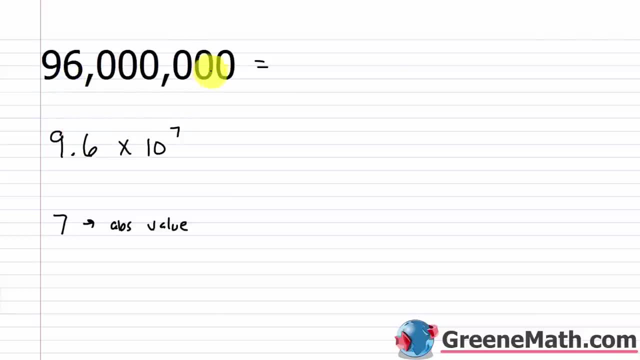 exponent, you're going to need to go through this. So if I'm here, 9.6, and I want to go to here, 96 million, what I need to multiply by a power of 10 that's going to tell me to move my decimal point to the right or the left. Remember, if this is positive, I'm going to be moving my decimal point to the right. If it's negative, I'm going to be moving my decimal point to the left. 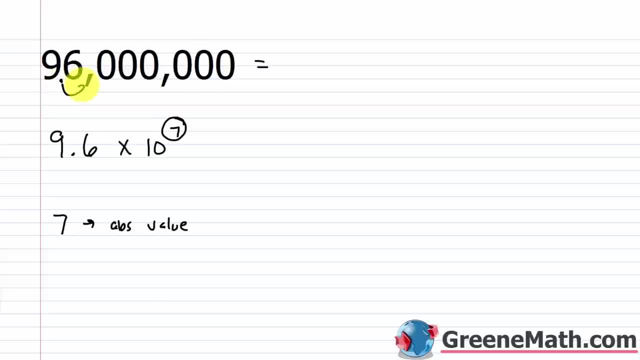 I want to move this 7 places to the right. I want to go 1, 2, 3, 4, 5, 6, 7 places to the right. So I can get back this original number. So I'm going to go 1, 2, 3, 4, 5, 6, 7 places to the right. I want to go 1, 2, 3, 4, 5, 6, 7 places to the left. So I can get back this original number 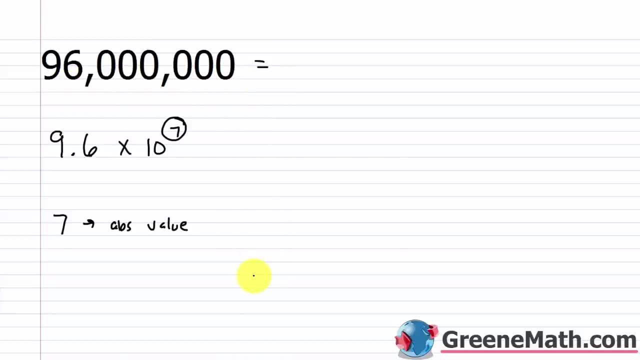 of 96 million. So 96 million written in scientific notation is 9.6 times 10 to the 7th power. 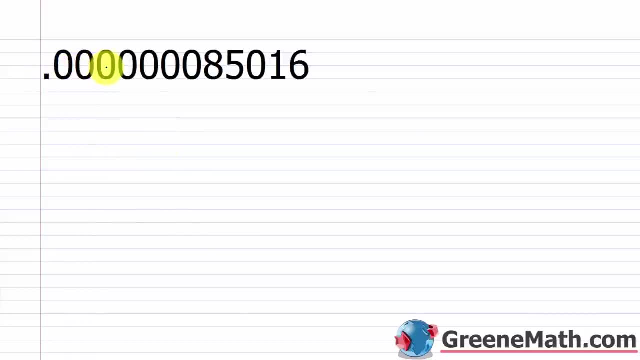 All right, let's take a look at this one. We have 0.00000085016. So I'm going to move this guy to immediately after the first non-zero digit. So after that 8, so it's going to end up right there. So this is going to be equal to, I'm going to have 8.5 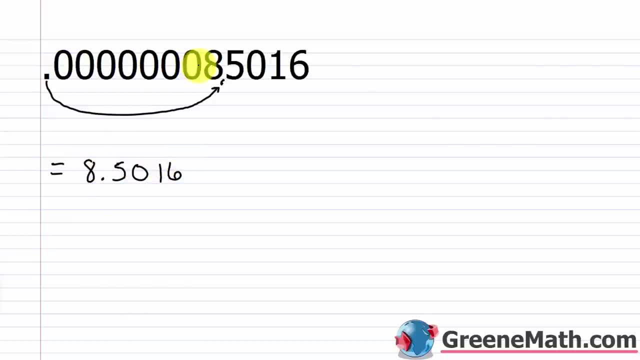 016. All the zeros that preceded that 8, I'm going to delete. I don't add any value to the number anymore. Then I'm going to multiply this by 10 raised to what power? Well, how far did I move the decimal point? 1, 2, 3, 4, 5, 6, 7, 8. Now, do I want 10 to the 8th power or 10 to the power of negative 8? Well, I clearly want 10 to the power of negative 8 because if I want to go from this right here, which is a large number, I'm going to have 10 to the power of negative 8. 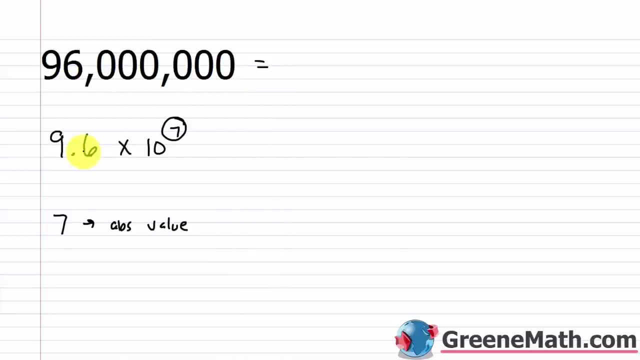 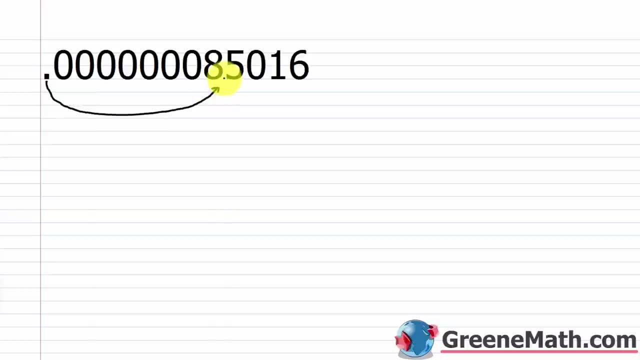 So I'm going to move this guy to immediately after the first non-zero digit, so after that 8.. So it's going to end up right there. So this is going to be equal to: I'm going to have 8.5016.. 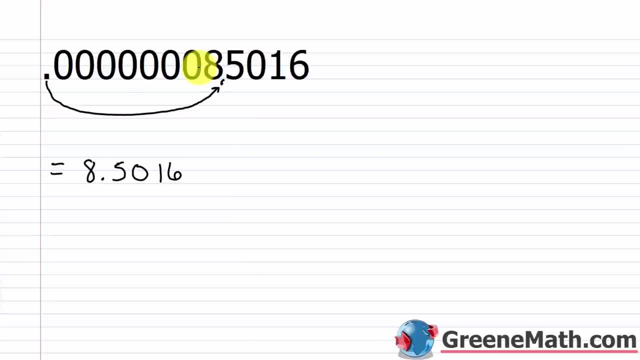 All the zeros that preceded that 8, I'm going to delete. I don't add any value to the number anymore. Then I'm going to multiply this by 10. raised to what power? Well, how far did I move the decimal point? 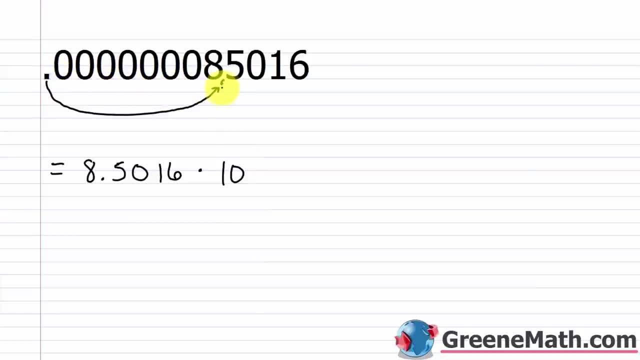 One, two, three, four, five, six, seven, eight. Now do I want 10 to the eighth power or 10 to the power of negative 8?? Well, I clearly want 10 to the power of negative 8, because, if I want to go from this right here, 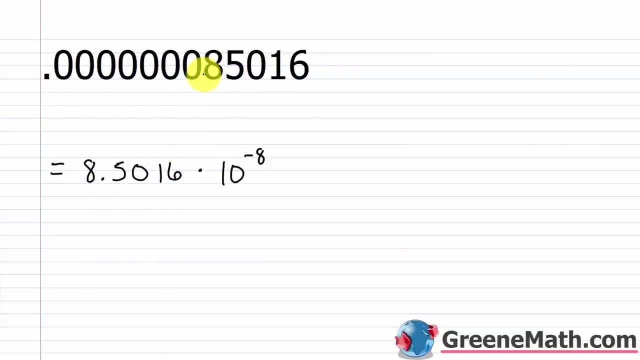 which is a larger number, to this, which is a smaller number. this decimal point has to move to the left. So this needs to be a negative 8, right, Because I want that decimal point to go to the left. So if I have this number, 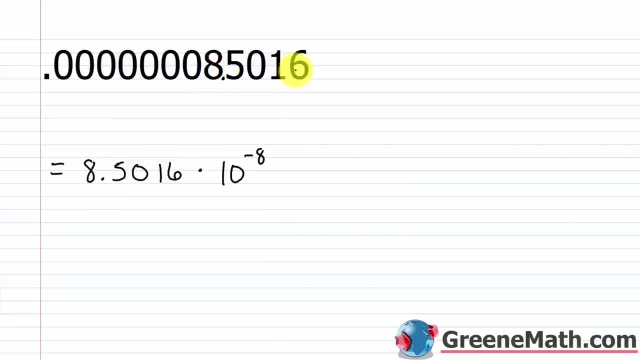 with this decimal point here, 8.5016, and I multiply it by 10 to the power of negative 8,. this is going to go one, two, three, four, five, six, seven, eight places to the left. 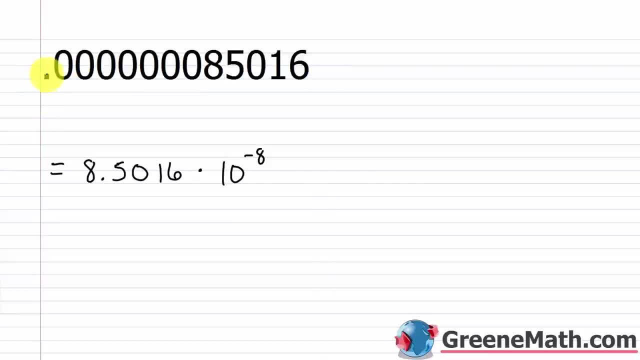 and put me right back where I started with this number, that's .0000008516.. What about 78,994,000,000,000?? Well, again I want to put my decimal point there to the left. put my decimal point there to the right. 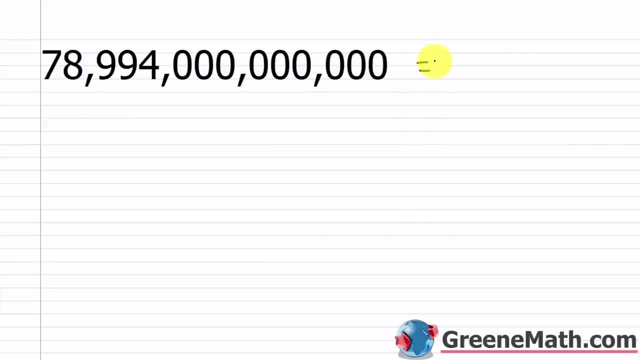 put my decimal point there, to the left decimal point, immediately after the first non-zero digit. So that's after that seven, And then I'm going to write the eight, the nine, the nine and then the four, These zeros I can. 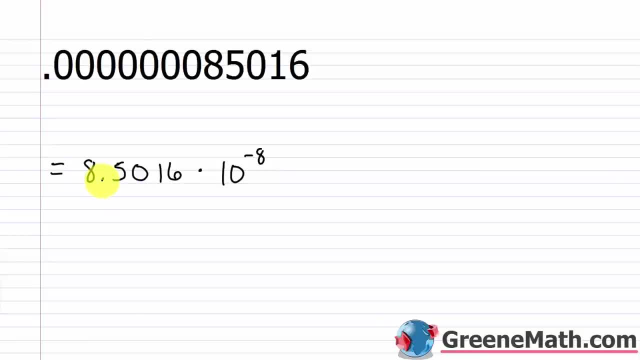 If I want to go from this larger number to this, which is a smaller number, this decimal point has to move to the left. So this needs to be a negative 8, right? Because I want that decimal point to go to the left. So if I have this number with this decimal point here, 8.5 016, and I multiply it by 10 to the power of negative 8, this is going to go 1, 2, 3, 4, 5, 6, 7, 8 places to the left. Put me right back where I started with this number that's 0.00085016. What about 78,994,000,000? Well, again, I want to put my decimal point immediately after 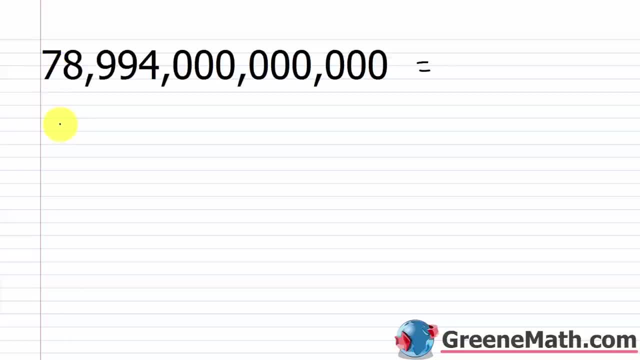 the first non-zero digit. So that's after that 7. And then I'm going to write the 8, the 9, the 9, and then the 4. These zeros, I can just delete. I don't need them. They don't add any value to the number now because my decimal point is here. Now, how far did I move the decimal point? Well, I went from here to here. So that's 1, 2, 3, 4, 5, 6, 7, 8, 9, 10, 11, 12, 13 places. 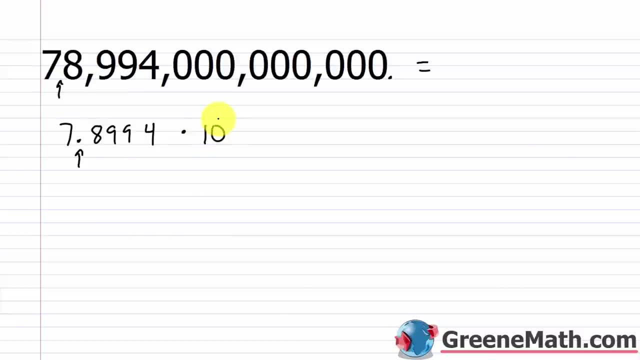 So times 10 to the power of, do I want positive 13 or negative 13? Well, again, this original number is bigger. So in order to get from the smaller value to the bigger value, I need that exponent to be positive. So this is going to be positive 13. So this will be 7, 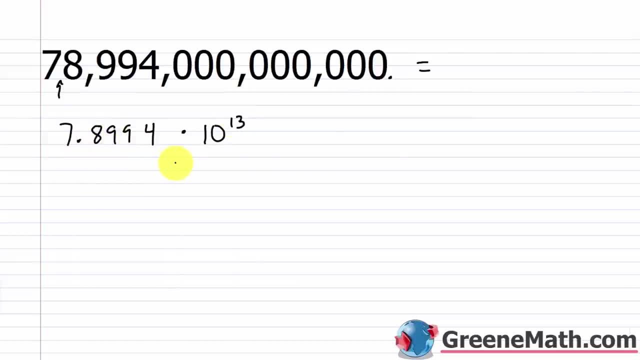 8, 9, 9, 4 times 10 to the 13th power. What about something like 0.321? Well, 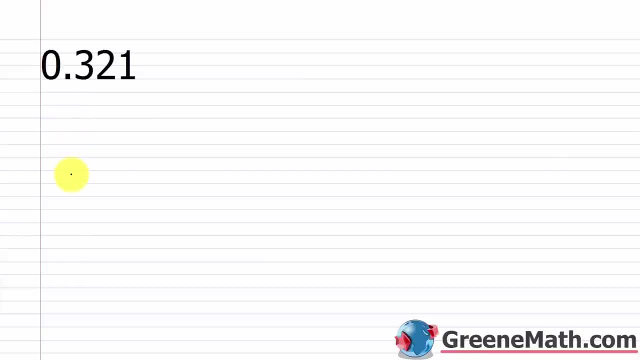 I'm going to move this decimal point to right after the first non-zero digit. First non-zero digit is a 3. So it's going to basically just go one place to the right. So this is going to be 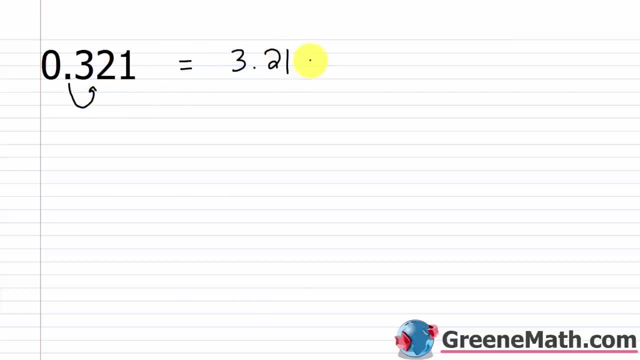 3.21. And then times 10, my exponent here is going to be negative 1. It went one place to the right. So I need to move it one place to the left to get back. So this is a bigger number, 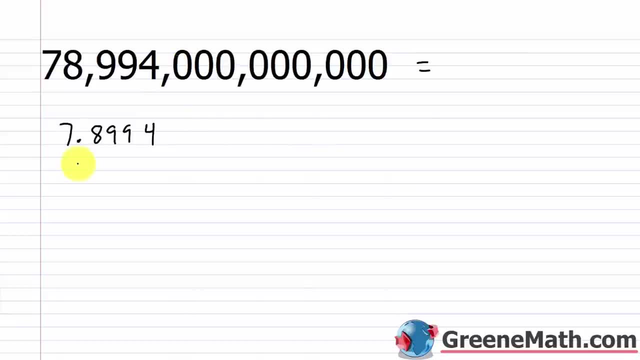 just delete. I don't need them. They don't add any value to the number now, because my decimal point is here. Now, how far did I move the decimal point? Well, I went from here to here, So that's 1,, 2,, 3,, 4,, 5,, 6,, 7,, 8,, 9,, 10,, 11,, 12,, 13 places. So times 10 to the power of. do I want positive? 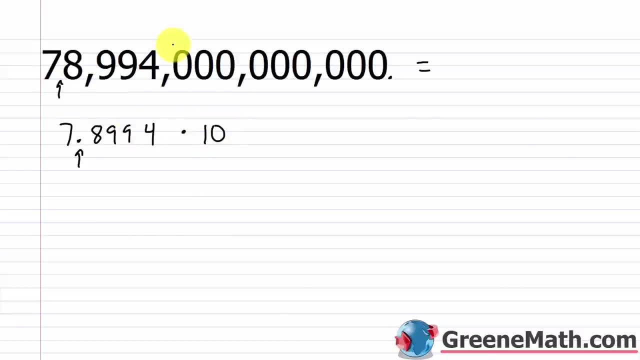 13 or negative 13?? Well, again, this original number is bigger. So in order to get from the smaller value to the bigger value, I need that exponent to be positive. So this is going to be positive 13.. So this will be 7.8994 times 10.. 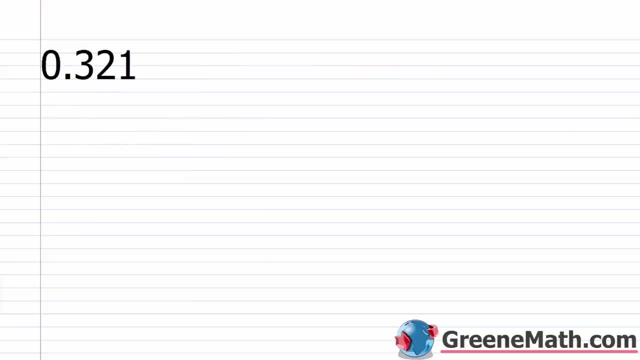 To the 13th power. What about something like 0.321?? Well, I'm going to move this decimal point to right after the first non-zero digit. First non-zero digit is a three, So it's going to basically just go one place to the right. So this is going to be 3.21.. And then times 10,. 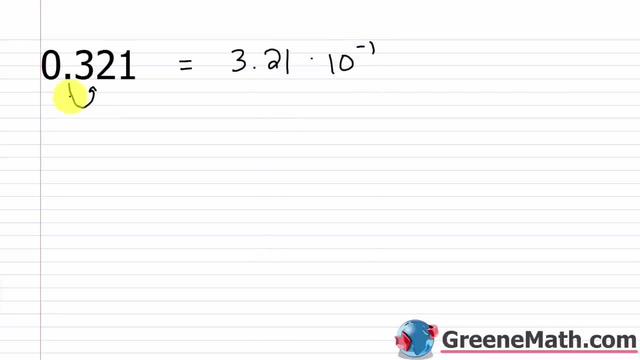 my exponent here is going to be negative one. It went one place to the right So I need to move it one place to the left to get back right. So 1.321.. This is a bigger number, the 3.21- than the original number, the 0.321.. So we need a negative. 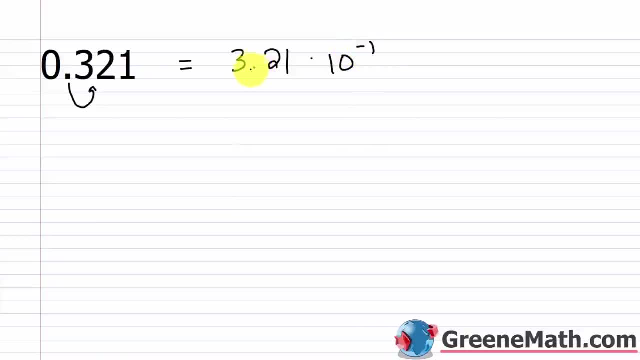 exponent- here Again, negative one tells me to take this decimal point and move this one place to the left. So we end up with 3.21 times 10. to the power of a negative one. All right, what about 15,065,000?? Again, put the decimal point immediately after the first non-zero digit, So 1.5065.. 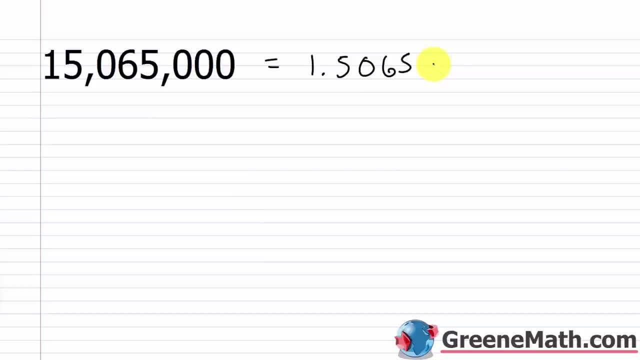 And I can delete those zeros. I don't need them. And then times 10 raised to what power? So we went 1,, 2,, 3,, 4, 5, 6, 7 places to the left. So in order to get back I need to go to the right, The original. 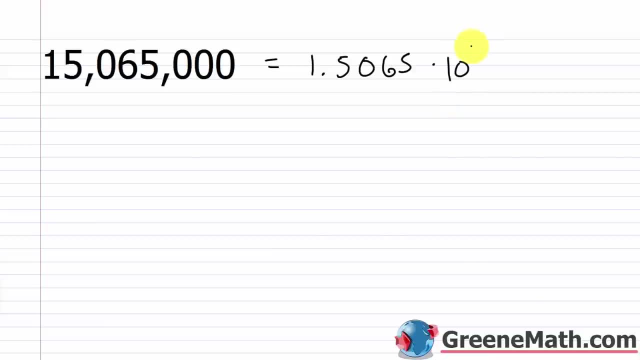 number is bigger, My exponent is going to need to be positive, So this would be 10 to the seventh power, right, Positive 7.. So you'd end up with 1.5065 times 10 to the seventh power. All right. 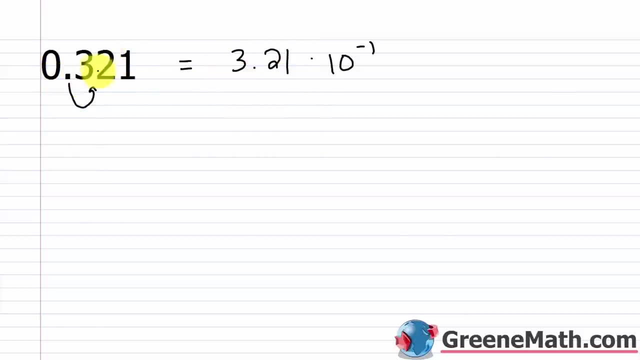 the 3.21, than the original number, the 0.321. So we need a negative exponent here. Again, negative 1 tells me to take this decimal point and move this one place to the left. 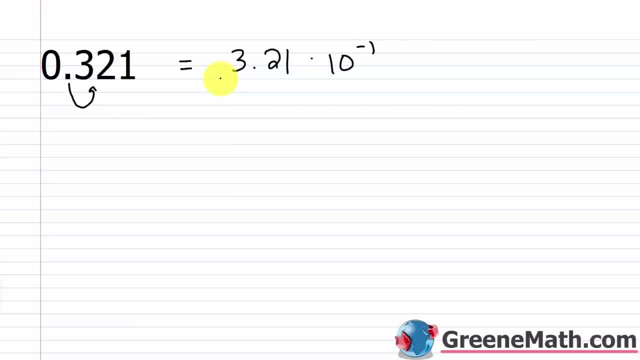 So we end up with 3.21 times 10 to the power of a negative 1. All right, what about 15,065,000? Again, put the decimal point immediately after the first non-zero digit. So 1.5065. And I can delete those zeros. I don't need them. And then times 10 raised to what power? So we went 1, 2, 3, 4, 5, 6, 7 places to the left. So in order to get back, I need to go to the right. The original number is bigger. My exponent is going to need to be positive. So this would be 10 to the 7th power, right? Positive 7. So you'd end up with 1.5065,000. 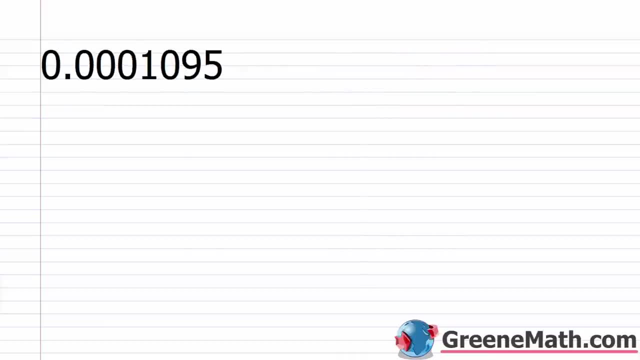 Times 10 to the 7th power. All right, let's take a look at 0.0001095. So again, move the decimal point to immediately after the first non-zero digit. It's going to go right there. So this would be 1.095. Then times 10 raised to what power? Well, this went 1, 2, 3, 4 places to the right. So then to get back there, I'd have to go 4 places to the left. So I want a negative 4 as my exponent. 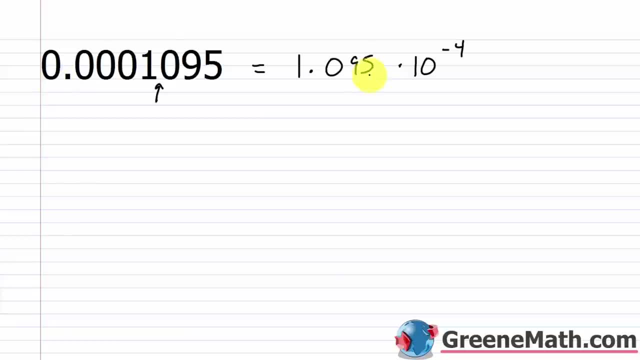 Again, if the original number is smaller than this number that I'm forming here, the exponent's going to be negative, right? So I end up with negative 4. If I took my decimal point there and I moved it 4 places to the left, 1, 2, 3, 4, I'd end up back with what I started with. So you get 1.095 times 10 to the power of negative 4. All right, so let's try writing a few without 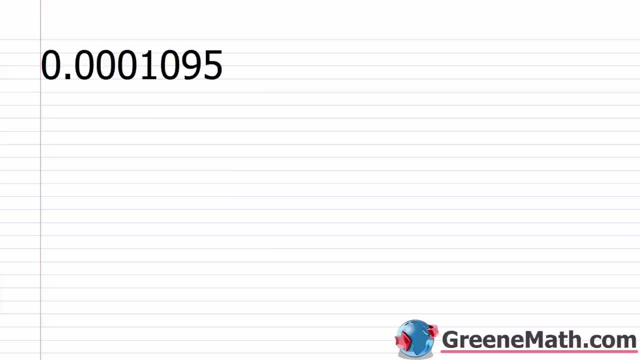 let's take a look at 0.5065.. 0.0001095.. So again, move the decimal point to immediately after the first non-zero digit. It's going to go right there. So this would be 1.095.. Then times 10 raised, to what power? Well? 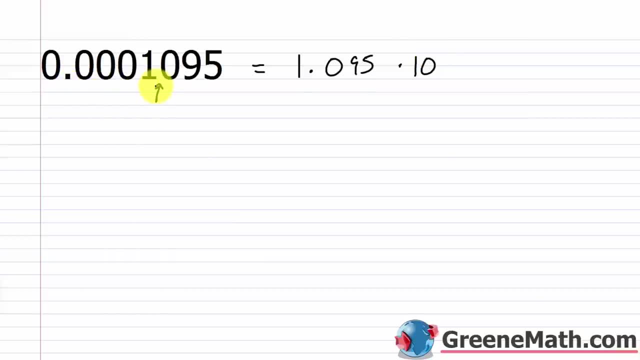 this went 1,, 2,, 3,, 4 places to the right. So then to get back there I'd have to go four places to the left. So I want a negative four as my exponent, Again, if the original number is smaller. 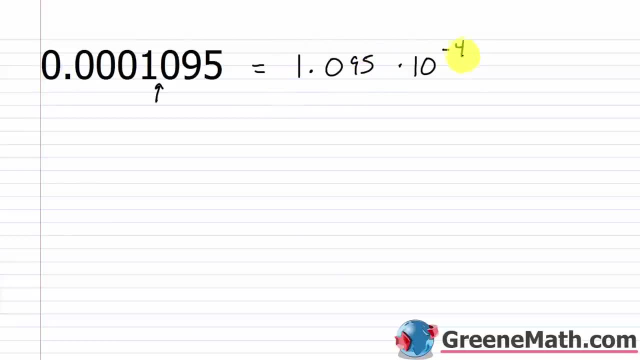 than the original number, I'm going to have to go to the left. So I'm going to have to go to the left And this number that I'm forming here, the exponent's going to be negative right. So I end up with negative four If I took my decimal point there and I moved it four places to the left. 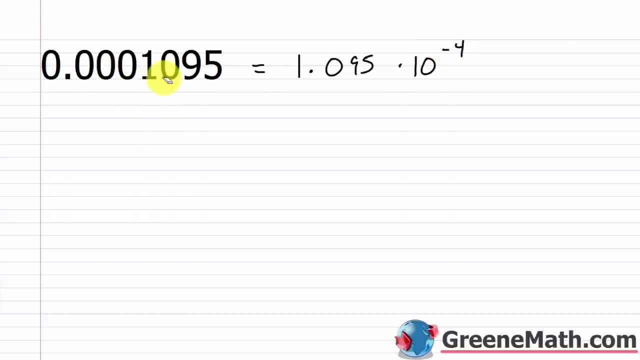 1, 2,, 3, 4, I'd end up back with what I started with. So you get 1.095 times 10 to the power of negative four. All right, so let's try writing a few without exponents. You want to go back and 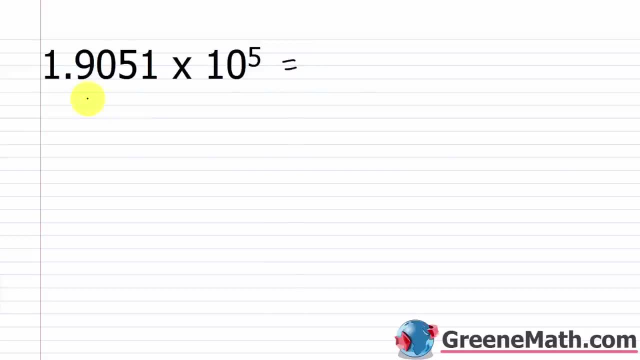 forth, get as much practice as you can, And so this would be- take this number here- 1.9051.. I'm multiplying by 10 to the fifth power, So I'm moving five places to the right. So let me add a. 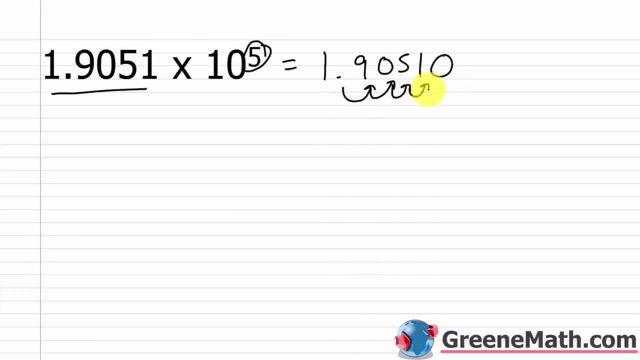 zero here. This is going to go 1,, 2,, 3,, 4, 5 places to the right And I'm going to end up with 190,510.. About 3.56 times 10 to the power of negative nine, So 3.56.. And I'm going to move. 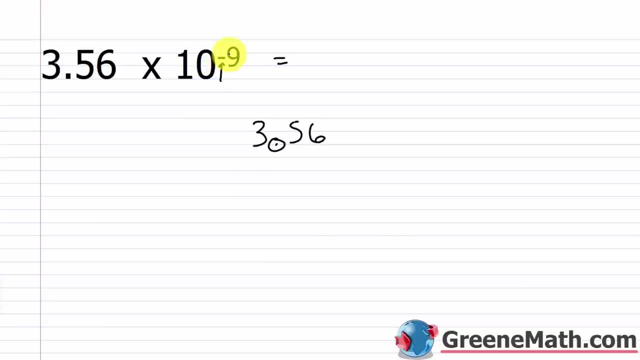 this decimal point nine places to the left. Again, that negative is telling me to go to the left, And the nine says nine spaces. So let me go ahead and put in eight zeros here: 1, 2,, 3,, 4,, 5,, 6,, 7,, 8.. This is going to go 1,. 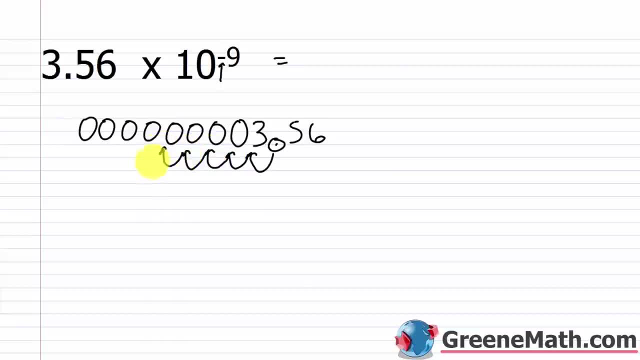 2,, 3,, 4,, 5,, 6,, 7,, 8,, finally nine, And so I'm going to end up with 0.00000000356 as my answer. What about 1.205 times 10?? 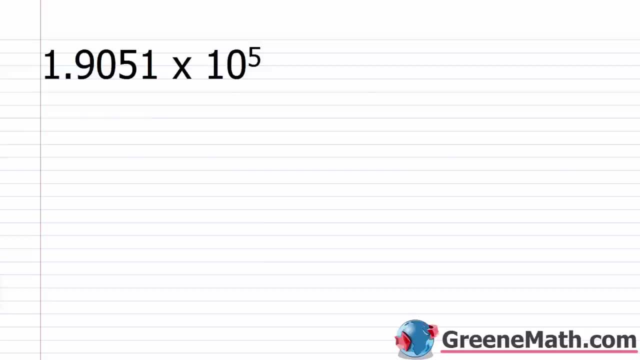 exponents. You want to go back and forth, get as much practice as you can. And so this would be, this number here, 1.9051. I'm multiplying by 10 to the fifth power. So I'm moving 5 places to the right. So let me add a zero here. This is going to go 1, 2, 3, 4, 5 places to the right. And I'm going to end up with 190,510. About 3.56 times 10 to the power of negative 9. So 3.56. And I'm 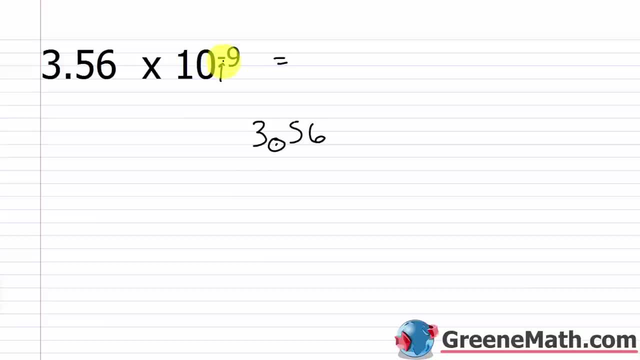 going to move this decimal point 9 places to the left. Again, that negative is telling me that I'm going to go to the left. And the 9 says 9 spaces. So let me go ahead and put in 8 zeros here. 1, 2, 3, 4, 5, 6, 7, 8. This is going to go 1, 2, 3, 4, 5, 6, 7, 8, finally 9. 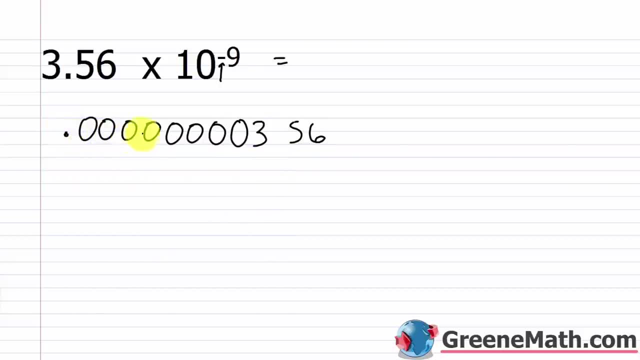 And so I'm going to end up with 0.000000356. As my answer. What about 1.205 times 10 to the third power? Well, again, just take this number, 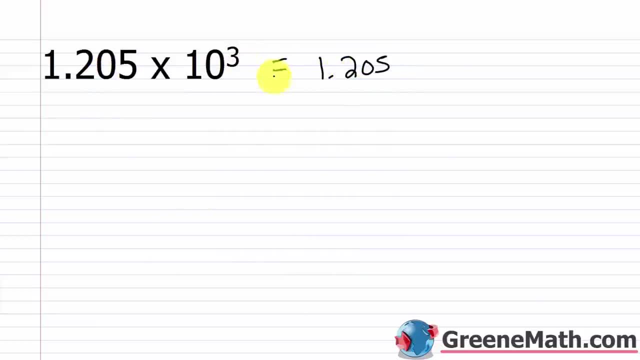 1.205. And we're going to move the exponent 3 places to the right. So 1, 2, 3. It's going to 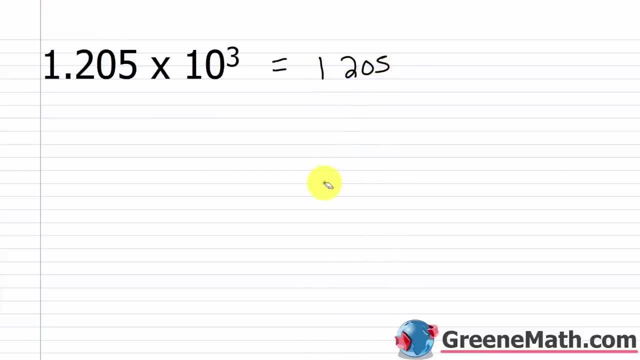 end up right there. You're going to end up with 1,205 as your answer. What about 6 times 10 to 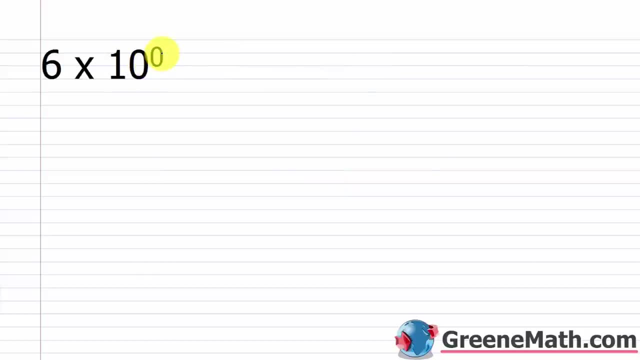 the power of 0? Well, we know anything to the power of 0 is 1. So this is basically 6 times 1 or 6. And just for future reference, this is how you're going to write a single, 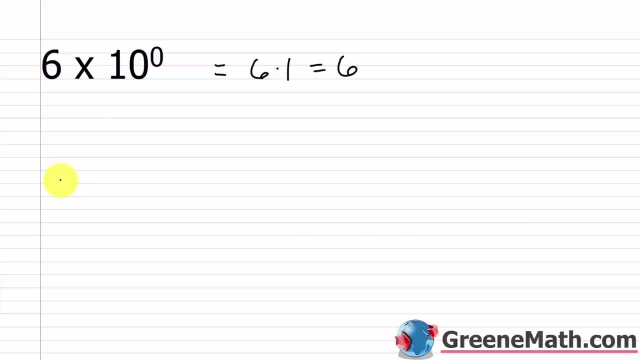 digit number in scientific notation. Your teacher might say, how do you write 4 in scientific notation? Well, you put 4 times 10 to the power of 0. Or how do you write 13 in 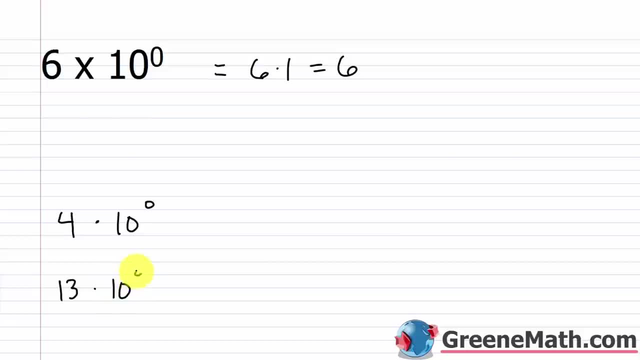 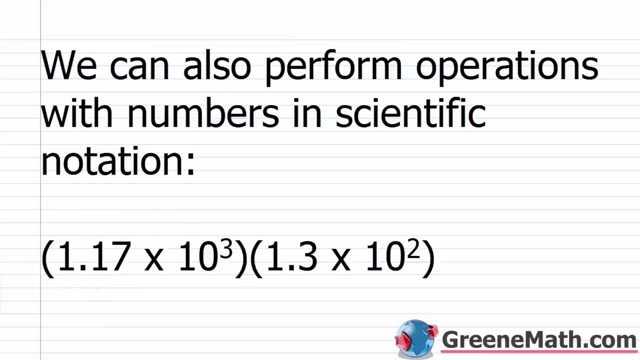 scientific notation? 13 times 10 to the power of 0. Because in each case, you're just multiplying by 1. Anything to the power of 0 other than 0 is 1. So we can also perform operations with numbers 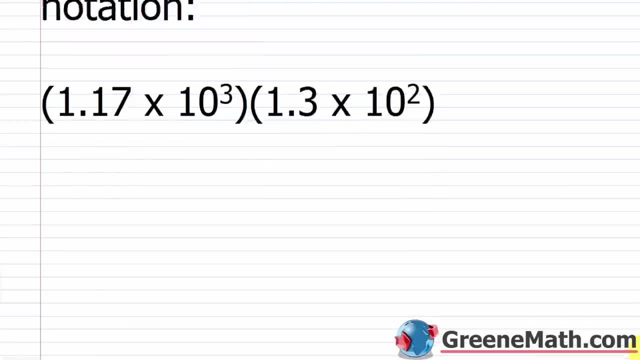 in scientific notation. There are different ways to kind of go about it. You have 1.17 times 10 cubed. 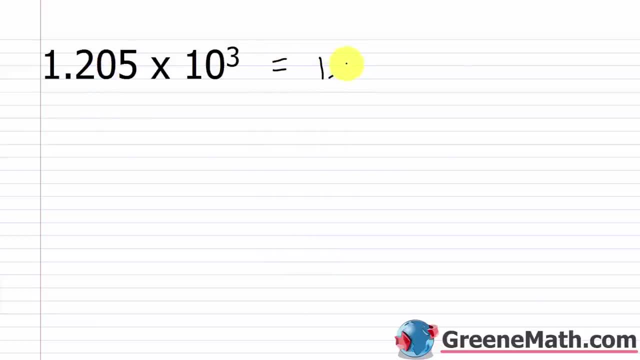 Well, again, just take this number: 1.205.. And we're going to move the exponent three places to the right, So 1,, 2, 3.. It's going to end up right there. You're going to end up with 1,205 as your. 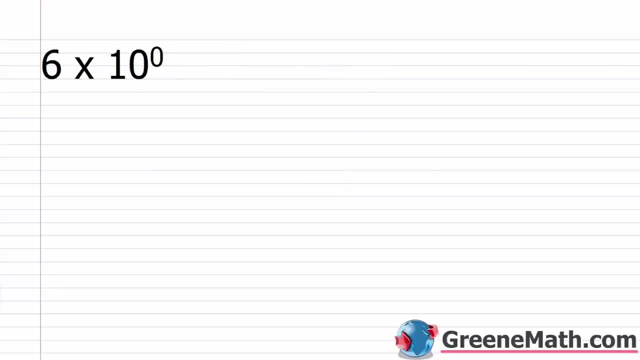 answer: What about 6 times 10 to the power of zero? Well, we know anything to the power of zero is one. So this is basically six times one or six. And just for future reference, this is how you're going to write a single digit number in scientific notation. Your teacher might say: 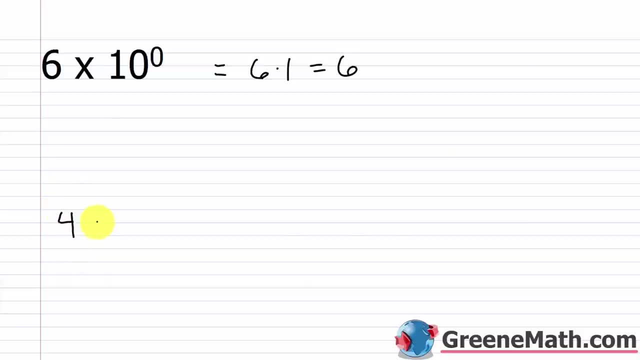 how do you write four in scientific notation? Well, you put four times 10 to the power of zero. Or how do you write 13 in scientific notation? 13 times 10 to the power of zero. Because in each case you're just multiplying by one right Anything to the power of zero other than zero. 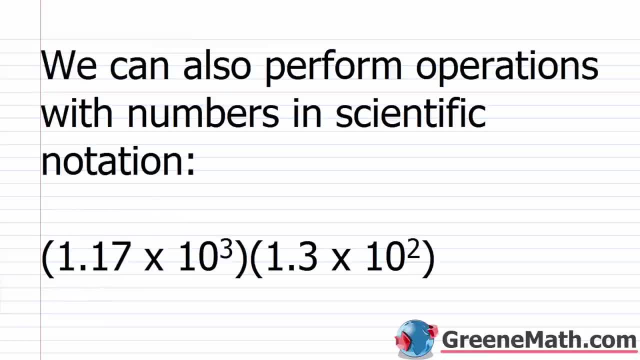 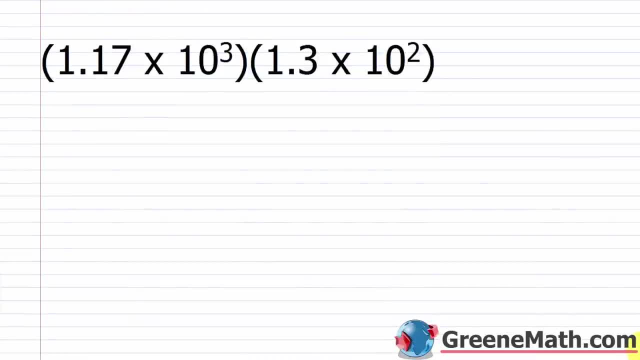 is one, So we can also perform operations with numbers in scientific notation. There are different ways to kind of go about it. You have 1.17 times 10 cubed times 1.3 times 10 squared. So kind of the simplest or the easiest way to do this is to say: okay, I have 1.17 times 1.3.. Kind of do. 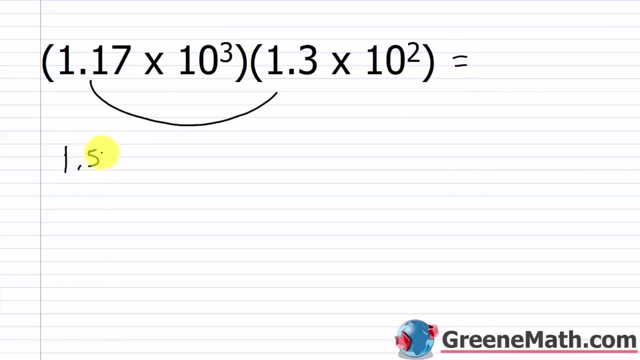 that first. That would give you 1.521.. Now, 10 cubed times 10 squared, you would use the product rule for exponents, So you'd have 10 as your base. that would stay the same: 3 plus 2 is 5.. So this: 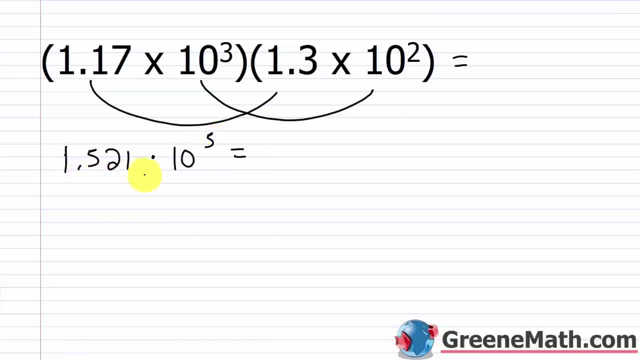 would end up being 1.521 times 10 to the fifth power. We know this would be 1.521.. Move the decimal point five places to the right, So let me put in the decimal point five places to the right, And so you're going to end up with 152,100.. All right? what about 2.7 times 10 to the power of? 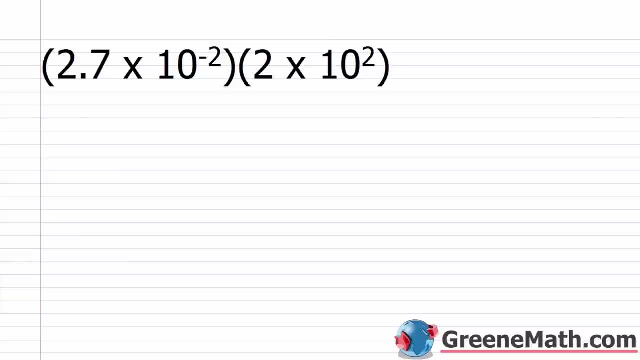 negative 2?. This is multiplied by 2 times 10 to the power of 2, or 2 times 10. squared Well, again you would multiply the numbers first 2 times 2.7.. That's going to give you 5.4.. And then, with this, 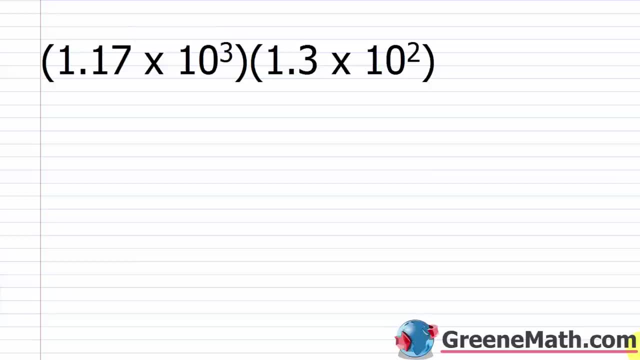 Times 1.3 times 10 squared. So kind of the simplest or the easiest way to do this is to say, okay, I have 1.17 times 1.3. Kind of do that first. That would give you 1.521. Now, 10 cubed times 10 squared, you would use the product rule for exponents. So you'd have 10 as your base that would stay the same. 3 plus 2 is 5. So this would end up being 1.521 times 10 to the 5th power. 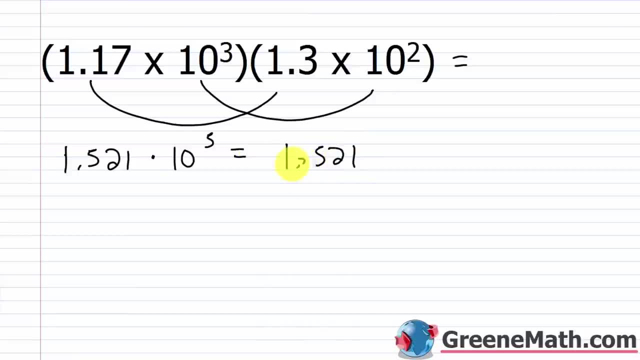 We know this would be 1.521. Move the decimal point five places to the right. So let me put in two zeros here. This would go 1, 2, 3, 4, 5 places to the right. And so you're going to end up with 152,100. All right. What 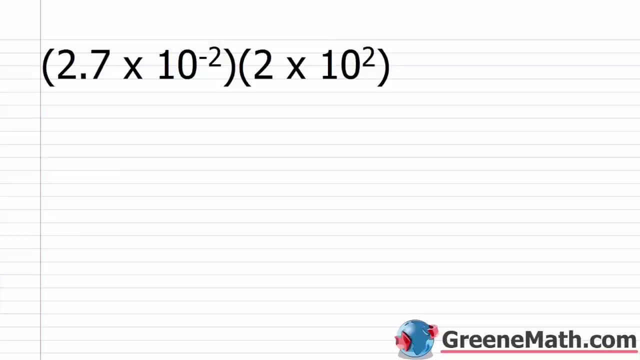 about 2.7 times 10 to the power of negative 2? This is multiplied by 2 times 10 to the power of 2, or 2 times 10 squared. Well, again, you would multiply the numbers first. 2 times 2.7. 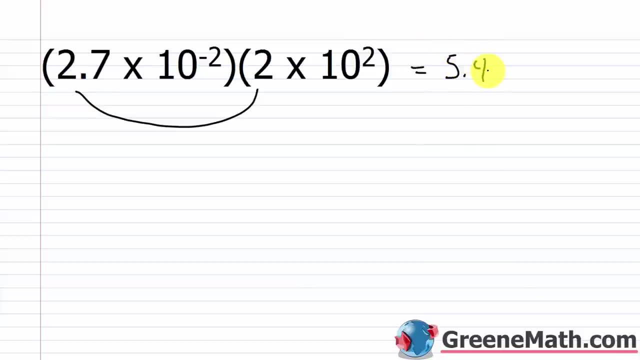 That's going to give you 5.4. And then with this one, you have 10 to the power of negative 2 times 10 squared. What is that really if you look at it? Well, that's 10 squared over 10 squared, or it's just 1. And you can see that using your product rule for exponents. You'd keep the base the same, which is 10. And you'd raise it to the power of negative 2 plus 2, which is 0. 10 to the power of 0 is 1. So this is really 5.4 times 1, which is 5.4. All right. What about 1.8 times 10 to the 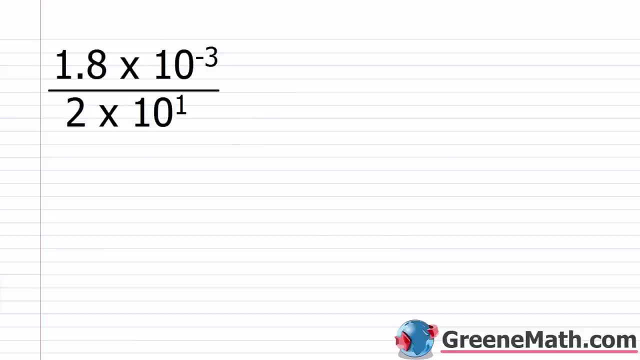 power of negative 3? 2 times 10 to the power of 1. So you could do 1.8 divided by 2 first. That would give you 0.9. And then you would multiply this by, use your quotient rule for exponents. You have 10 to the power of negative 3 over 10 to the power of 1. So times 10 to the power of negative 3 minus 1. So this would be equal to 0.9 times, you'd have 10 raised to the power of negative 3 minus 1 is negative 4. So then to completely finish this off, you'd have 0.9. If I have 10 to the power of negative 4, I need to move this four places to the left. So 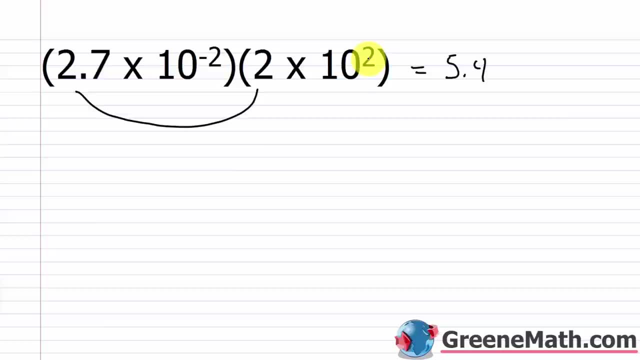 one, you have 10 to the power of negative 2.. So you would multiply the numbers first 2 times 2.7.. 2 times 10 squared. What is that really? if you look at it? Well, that's 10 squared over 10. 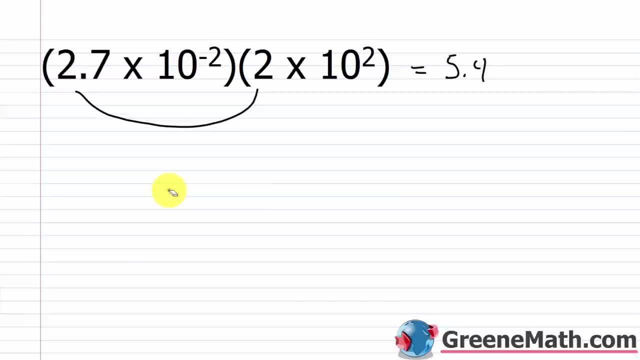 squared or it's just 1.. You can see that, using your product rule for exponents, You'd keep the base the same, which is 10.. And you'd raise it to the power of negative 2 plus 2, which is 0.. 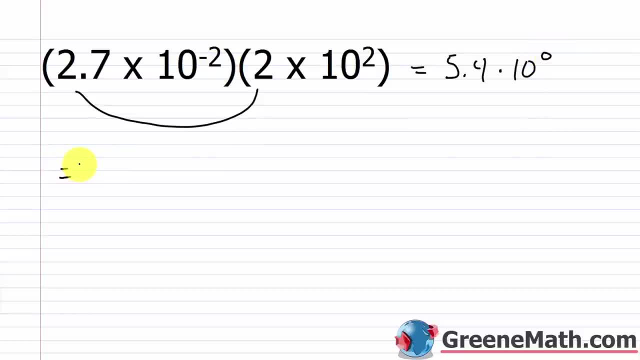 10 to the power of 0 is 1.. So this is really 5.4 times 1, which is 5.4.. All right, what about 1.8 times 10 to the power of negative 3 over 2 times 10 to the power of 1?? So you could do 1.8 divided. 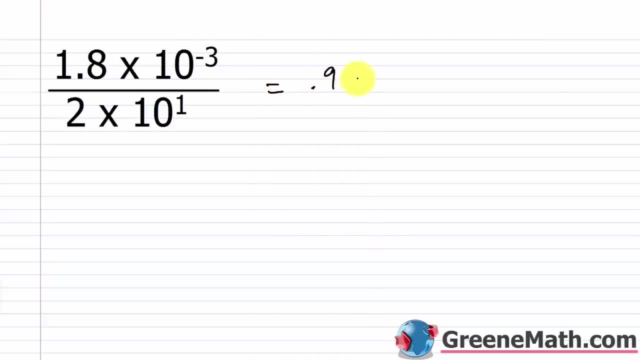 by 2. first That would give you 0.9.. And then you would multiply this by use your quotient rule for exponents. You have 10 to the power of negative, 3 over 10 to the power of 1.. So times 10 to the. 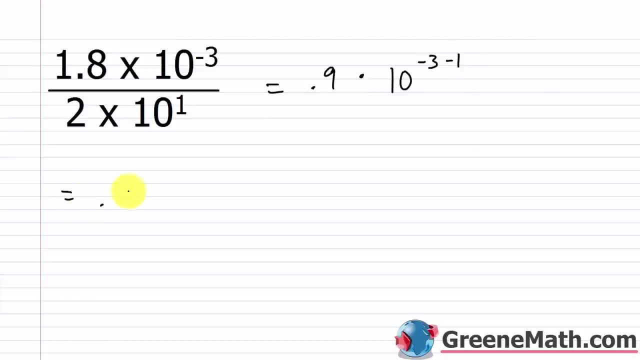 power of negative 3 minus 1.. So this would be equal to 0.9 times. you would have 10 raised to the power of negative 3 minus 1 is negative 4.. So then, to completely finish this off, you'd have: 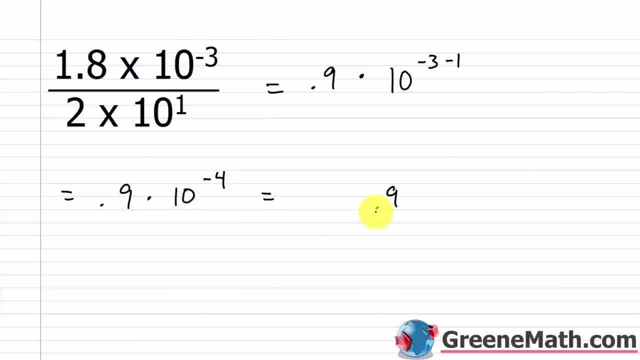 0.9.. If I have 10 to the power of negative 4, I need to move this four places to the left. So let me put 1,, 2,, 3, 4 zeros in. This would go 1,, 2,, 3,, 4 places to the. 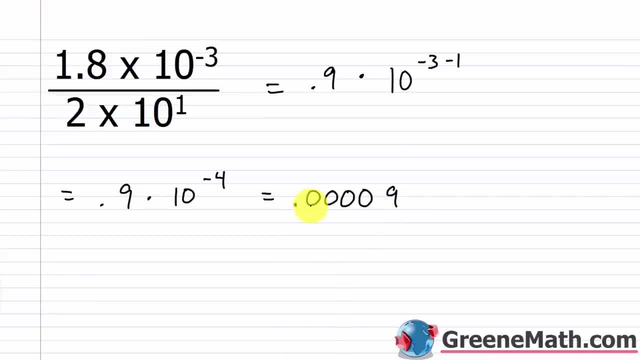 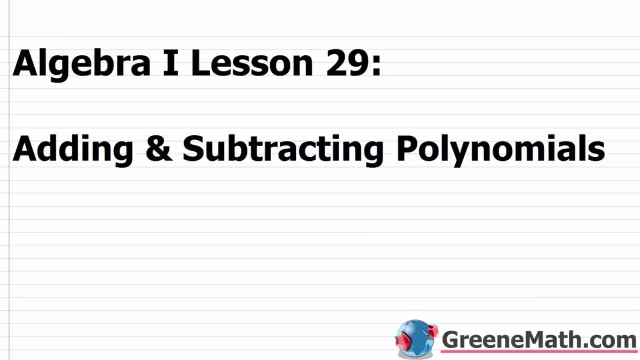 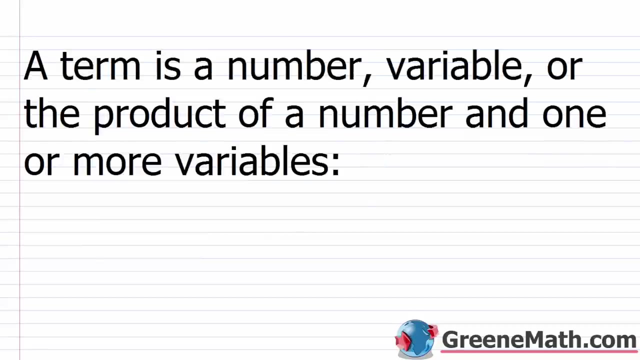 left, So I'd end up with 0.0009 as my answer. Hello and welcome to Algebra 1, Lesson 29.. In this video, we're going to learn about adding and subtracting polynomials. All right, so we're going to start out today by just talking about some basic vocabulary. So we previously 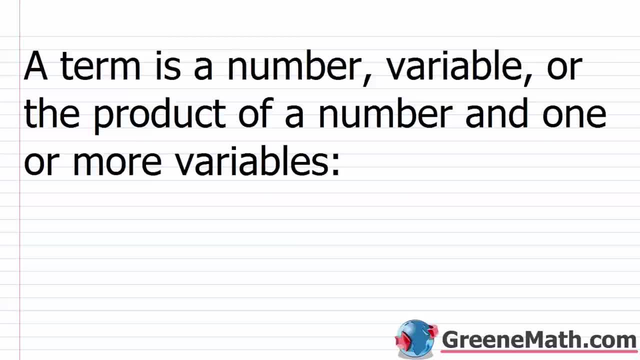 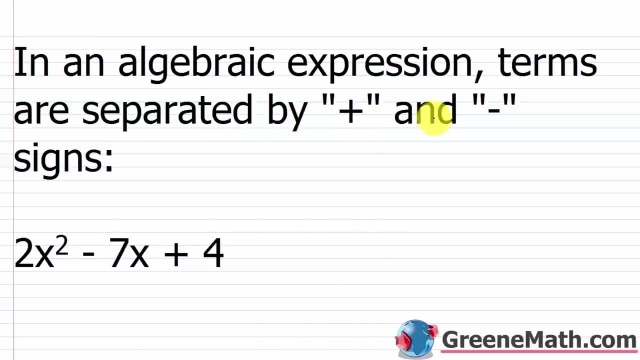 learned the definition for a term, So recall that a term is a number, a variable or the product of a number and one or more variables. So, as you may recall, in an algebraic expression terms are separated by plus and minus signs. So 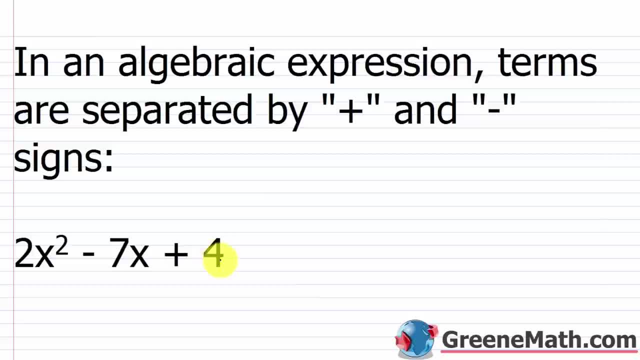 for example, we have 2x squared minus 7x plus 4.. So this is a term, this 2x squared, And then we have a minus sign, This is a term, this 7x, And we have a plus sign, And then this 4 is a term. So notice how this is a barrier. 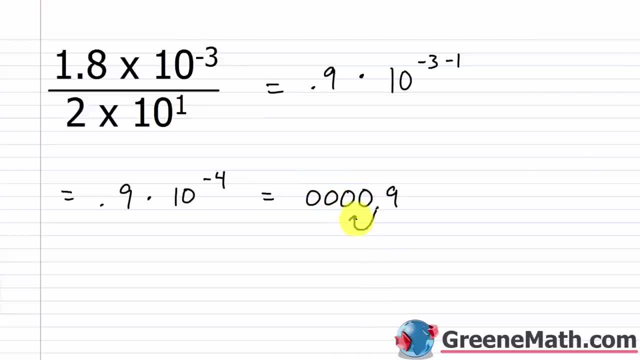 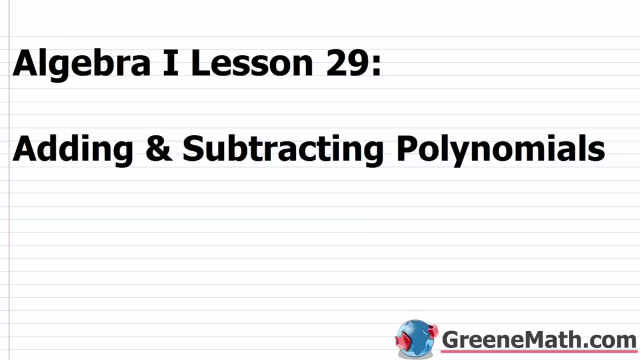 let me put 1, 2, 3, 4 zeros in. This would go 1, 2, 3, 4 places to the left. So I'd end up with 0.0009 as my answer. Hello and welcome to Algebra 1 Lesson 29. In this video, we're going to learn 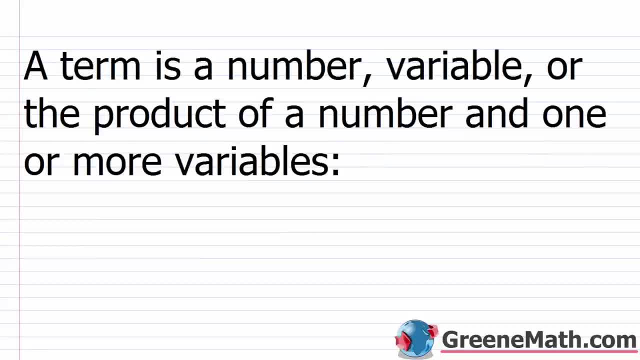 about adding and subtracting polynomials. All right. So we're going to start out today by just 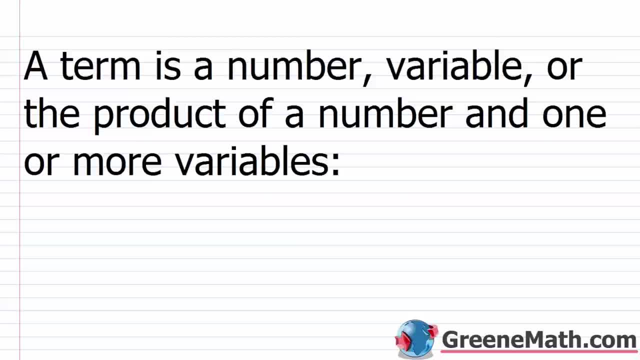 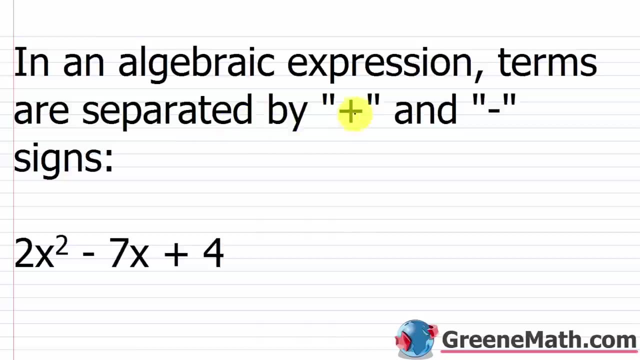 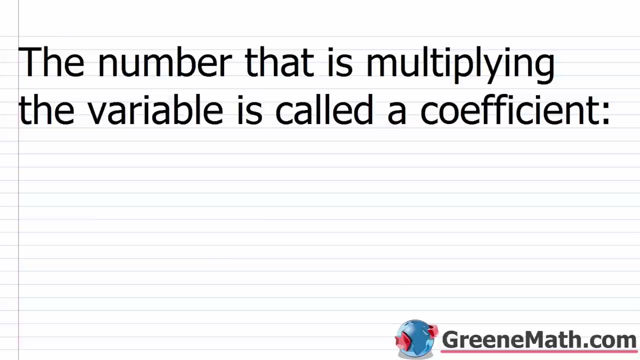 adding a few things. So we previously learned the definition for a term. So recall that a term is a number, a variable, or the product of a number and one or more variables. So as you may recall, in an algebraic expression, terms are separated by plus and minus signs. So for example, we have 2x squared minus 7x plus 4. So this is a term, this 2x squared. We have a minus sign. This is a term, this 7x. And we have a plus sign. And then this 4 is a term. So notice how this is a barrier, right, between your terms. So you have the term 2x squared, the term 7x, and then the term 4. All right. So I also want you to recall that the number that is multiplying the variable is called a coefficient. So for example, if I have something like 3x to the fifth power, the 3 that's multiplying this x to the fifth power is known as the coefficient. 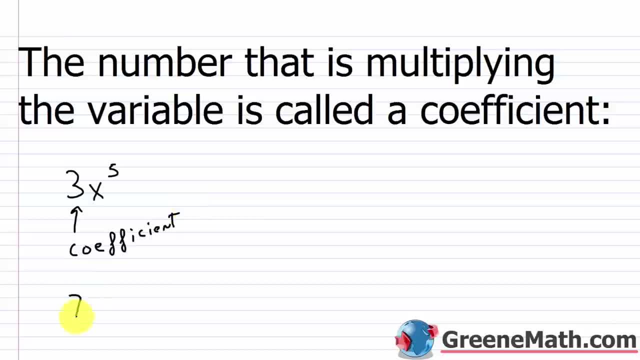 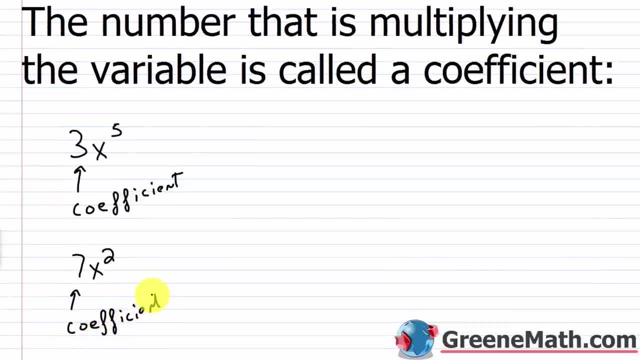 Or as another example, you could have, let's say, 7x squared. 7 is the coefficient. And again, I just give you these definitions because I'm going to be referring to things later on. I might say, hey, just add the coefficients together. So you need to know, what I'm talking about. All right. So now let's talk again about like terms. 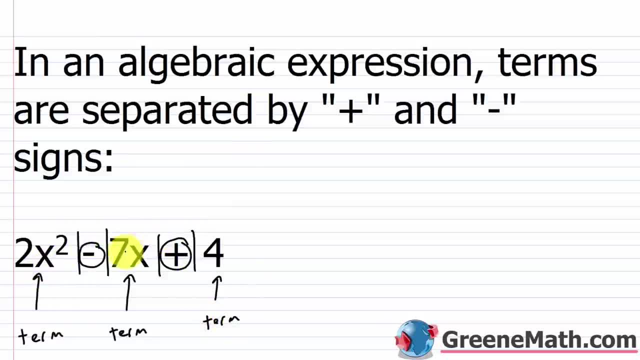 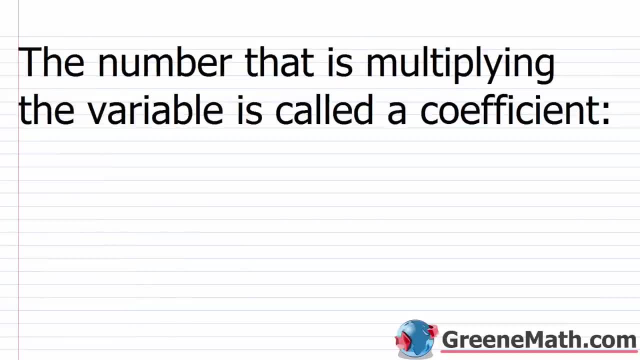 right between your terms. So you have the term 2x squared, the term 7x and then the term 4.. All right, so I also want you to recall that the number that is multiplying the variable is called a coefficient. So, for example, if I have something like 3x to the fifth power, 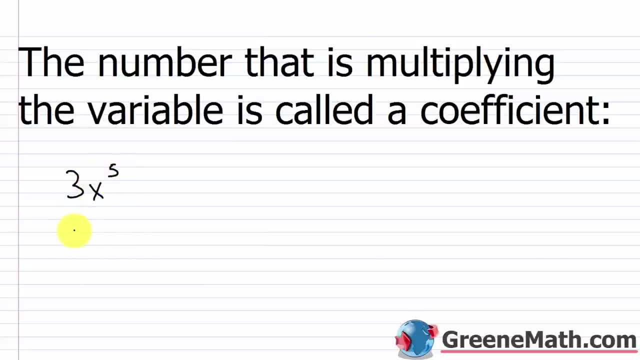 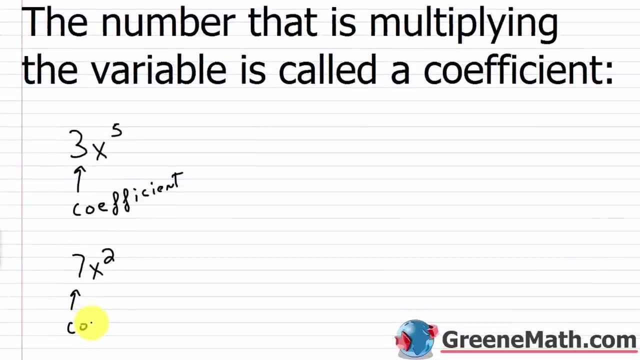 the 3, that's multiplying this x to the fifth power, is known as the coefficient. Or as another example you could have, let's say, 7x squared 7 is the coefficient. And again, I just give you these definitions because I'm going to be referring to 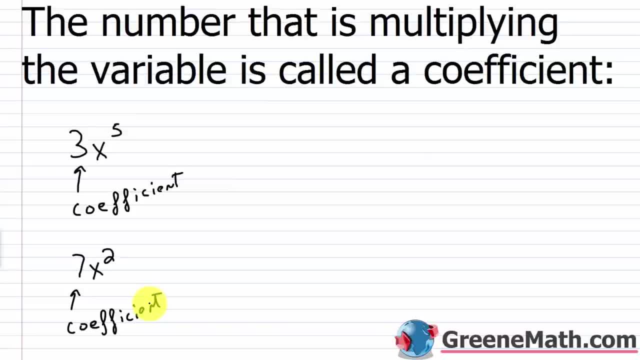 things later on, I might say, hey, just add the coefficients together. So you need to know what I'm talking about. All right, so now let's talk again about like terms. So what we're going to do is we're going to talk about like terms. 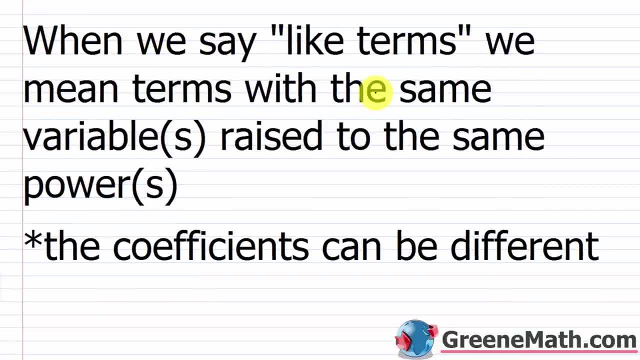 So when we say like terms, we mean terms with the same variable or variables raised to the same power or powers. So the coefficients can be different, but that's the only thing that can differ. So let me give you some examples. Here we have 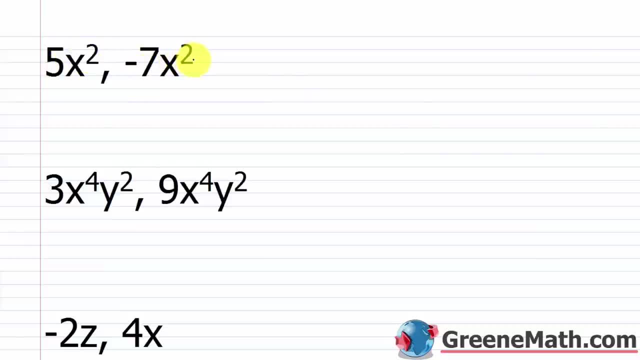 5x squared and we have negative 7x squared. So these are like terms. These are like terms Again. look at the variable- This is an x and this is an x- And then look at the power that it's raised to. And then look at the power that it's raised to And then look at the power that. 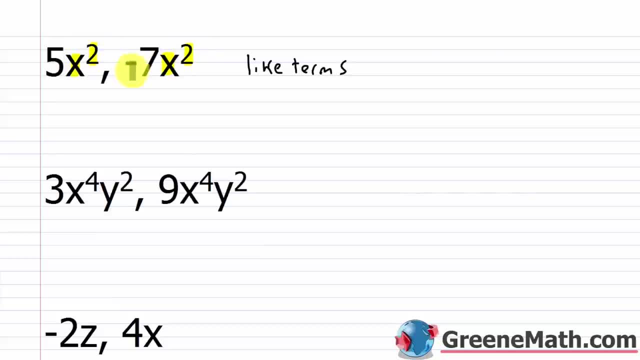 it's raised to. This is raised to the second power, and so is this. The coefficients are different, right, If I highlight that in a different color? this one is 5, and this one is negative 7,, but that's okay. Again, same variable or variables if you have more than one. 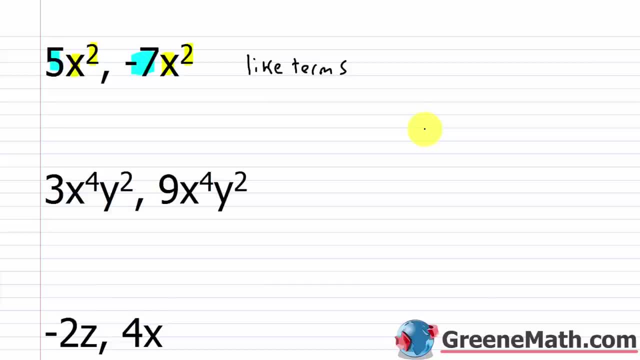 raised to the same power, or could be powers again. if you're dealing with one of those situations, All right, let's look at this one. right here We have 3x to the fourth power y squared. Then we have 9x to the fourth power y squared. 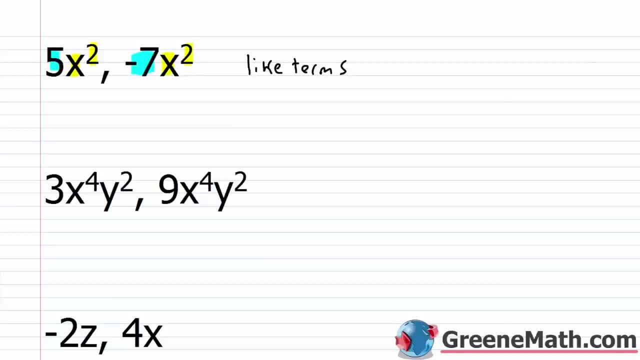 Again, these are like terms. If you look at the variables again, we have two here now. We have x and we have x, We have y and we have y. Now you're looking at the powers. We have x to the fourth power, x to the fourth power. We have y squared and y squared. So these are like. 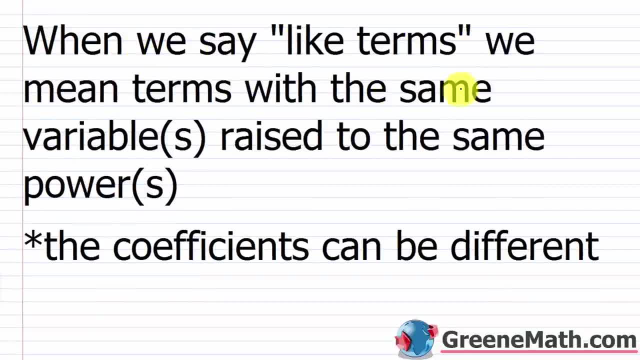 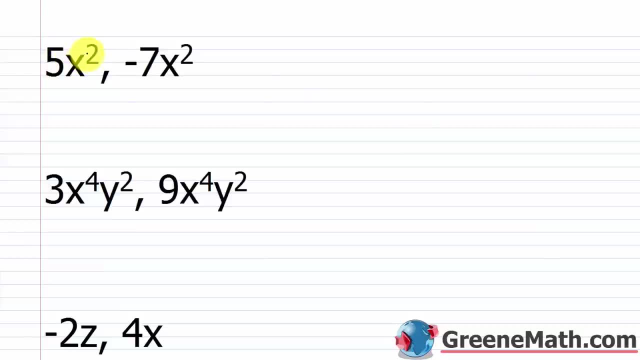 So when we say like terms, we mean terms with the same variable or variables raised to the same power or powers. So the coefficients can be different. But that's the only thing that can differ. So let me give you some examples. Here we have 5x squared, and we have negative 7x squared. So these are like terms. These are like terms. Again, look at the variable. This is an x, and this is an x. And then look at the power that it's raised to. This is raised to the second power, and so is this. The coefficients are different, right? If I highlight that in a different color, this one is 5, and this one is negative 7. But that's OK. Again, same variable or variables, if you have more than one, raised to the same power or could be powers, again, 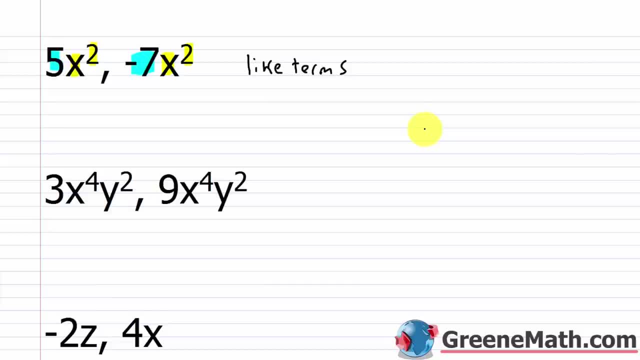 if you're dealing with one of those situations. All right. Let's look at this one right here. 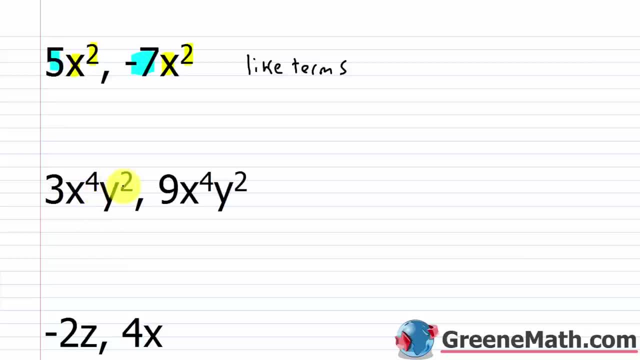 We have 3x to the fourth power, y squared, and we have 9x to the fourth power, y squared. So again, these are like terms. If you look at the variables, again, we have two here now. We have x, and we have x. We have y, and we have y. Now you're looking at the powers. We have x to the fourth power, x to the fourth power. We have y squared, and y squared. So these are like terms. And let's say you've got a situation where you 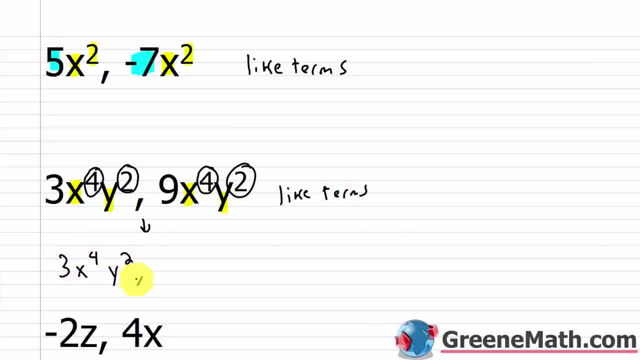 3x to the fourth power, y squared. And then this differed by just a little bit. Let's say it was 9x cubed, y squared. These are not like terms. Not like terms. Because this right here, this is x cubed, and this is x to the fourth power. So everything in terms of your variable and the power that it's raised to has to be exactly the same. It can't differ even by a little bit. 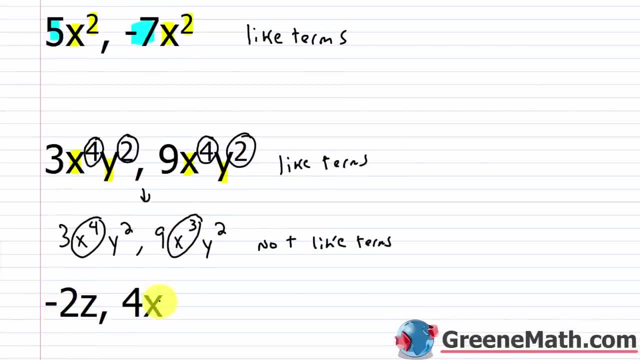 So in this example here, where we have negative 2, z, and 4x, obviously those aren't like terms. They don't even have the same variable. This one has a variable of z. This one has a variable of x. So these are not like terms. All right, 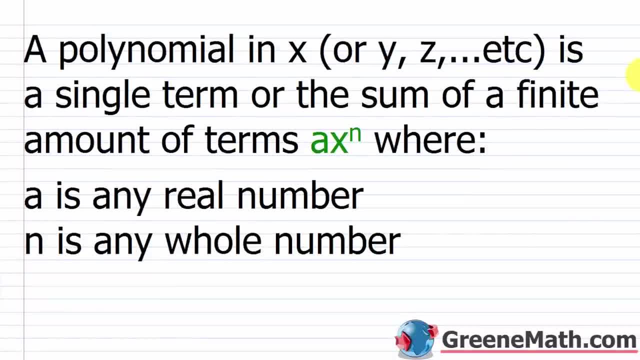 so let me give you the textbook definition for a polynomial now. And you're going to read this, and it's going to be a little bit confusing at first. And hopefully I can give you a little insight into kind of how you can look at the examples and say, this is a polynomial, and this is not a polynomial. So a polynomial in x, 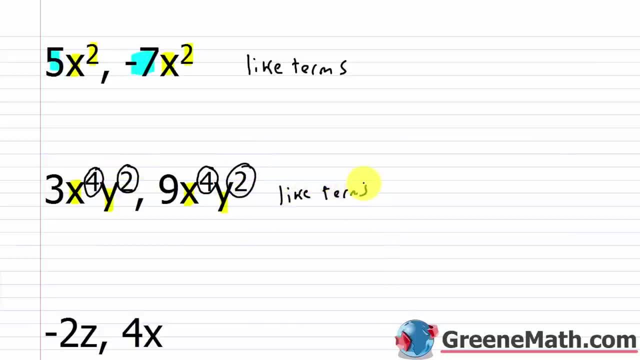 terms. And let's say you've got a situation where you had something like 3x to the fourth power y squared. Then this differed by just a little bit. Let's say it was 9x cubed y squared. These are not. 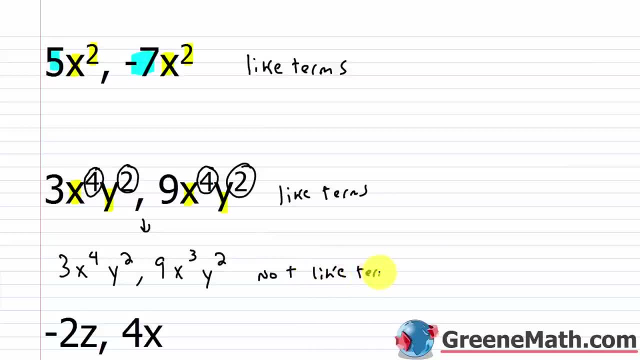 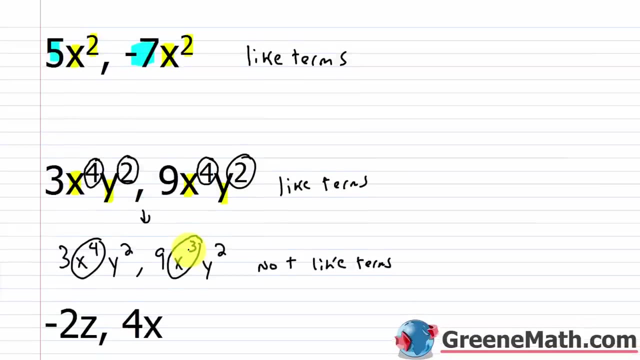 like terms, Not like terms, Because this right here, this is x cubed and this is x to the fourth power. So everything in terms of your variable and the power that it's raised to, has to be exactly the same. It can't differ even by a little bit. So in this example here, where we have negative 2z, 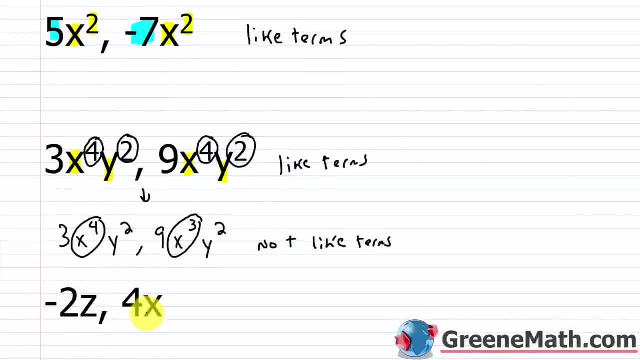 and 4x. obviously those aren't like terms, right? They don't even have the same variable. This one has a variable of z, This one has a variable of x. So these are not like terms. All right, So let me give you the textbook definition for a polynomial now. And 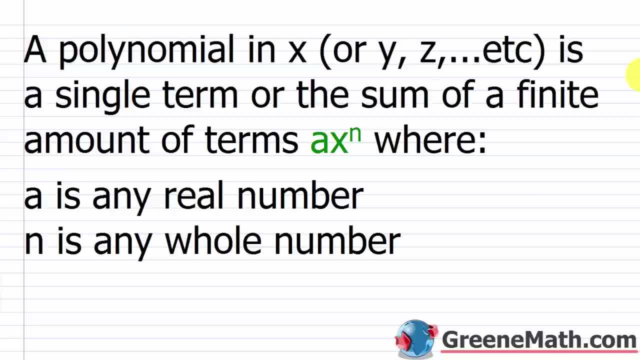 you're going to read this And it's going to be a little bit confusing at first And hopefully I can give you a little insight into kind of how you can look at the examples and say this is a polynomial and this is not a polynomial, So a polynomial in x or it could be another. 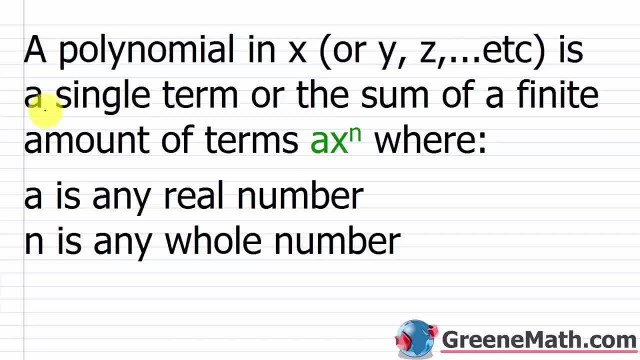 variable like y or z. whatever you want is a single term or the sum of a finite right. Finite means it has an end amount of terms, ax to the power of n, where a is any real number and n is any whole number. So what they're saying is that 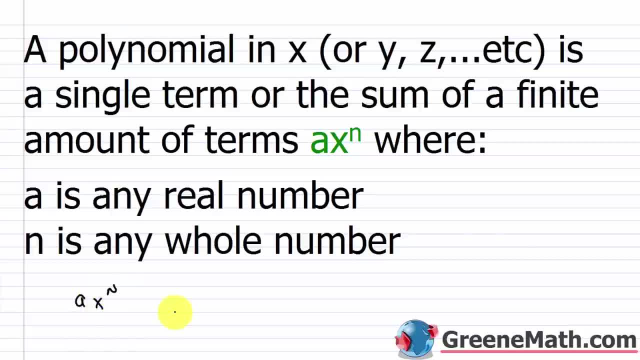 we have ax to the power of n. a is any real number, So anything you could think of can be plugged in for a. It could be a negative, It could be a positive, It could be a fraction, It could be. anything you could think of can be plugged in there. So any 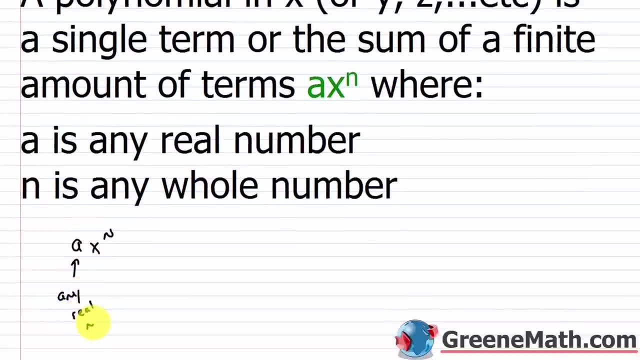 real number, Any real number. x is the variable, So that doesn't have to be x, As I just said up here. it could be y or z or w, whatever you want to use for that. And then n is the exponent on x. 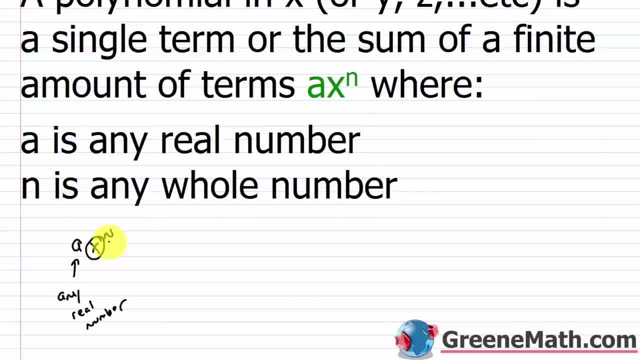 And it says that it has to be a whole number, So it can be 0.. It can be 1.. It can be 2, something like that. So what you want to pay attention to is that you're going to be able to. 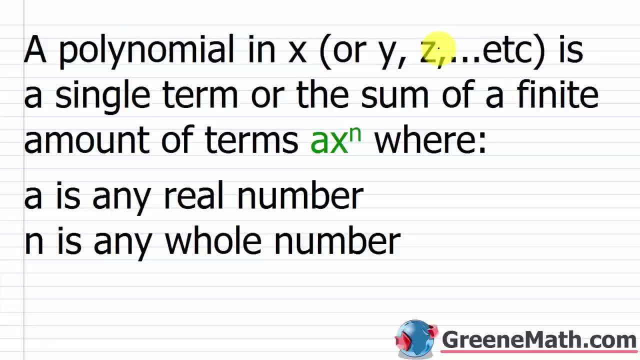 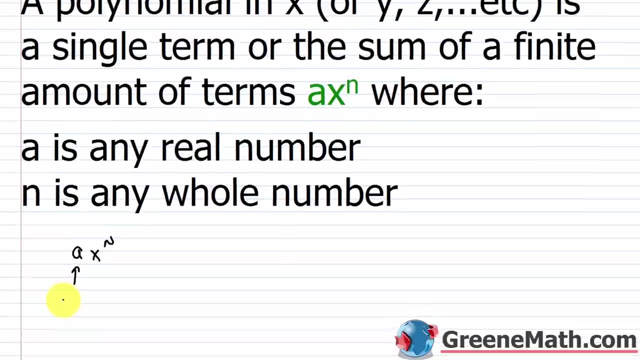 or it could be another variable like y or z, whatever you want, is a single term or the sum of a finite, right? Finite means it has an end, amount of terms ax to the power of n, where a is any real number, and n is any whole number. So what they're saying is that we have ax to the power of n. a is any real number. So anything you could think of can be, plugged in for a. Could be a negative, could be a positive, could be a fraction, could be anything you could think of can be plugged in there. So any real number, any real number. x is the variable. 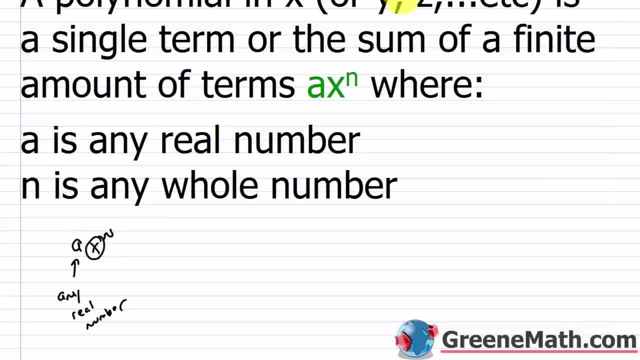 So that doesn't have to be x. As I just said up here, it could be y or z or w, whatever you want to use for that. And then n is the exponent on x, and it says that it has to be a whole number. So it can be zero, it can be one, it can be two, it can be three, it can be four, it can be five, one, it can be two, something like that. So what you want to pay attention for, you want to look for negatives, and you want to look for fractions and things that are not whole numbers. If you see that, if you see that in place here, you don't have a polynomial, okay? You don't have a polynomial. 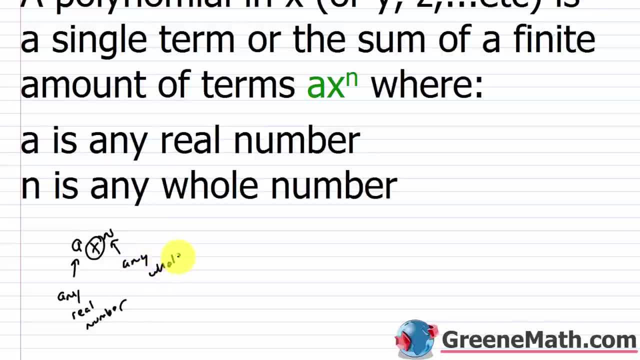 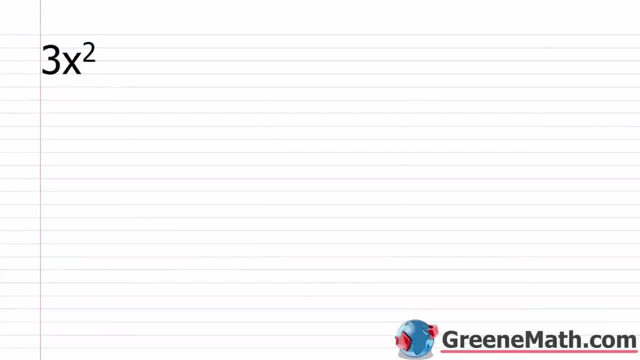 So this, any whole number. So let me give you an example. We have something here, 3x squared, okay? And remember, we're looking for a, 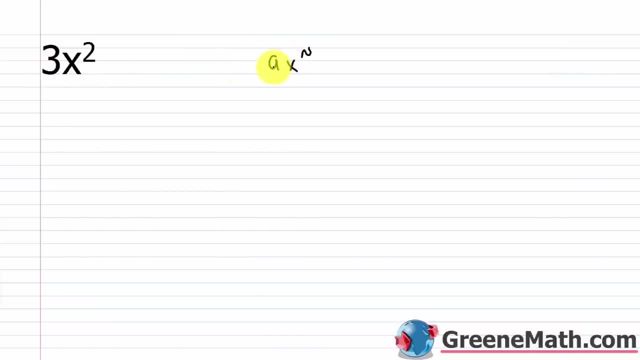 x to the power of n. So a can be any real number, and so 3 here is representing a. So that's fine. 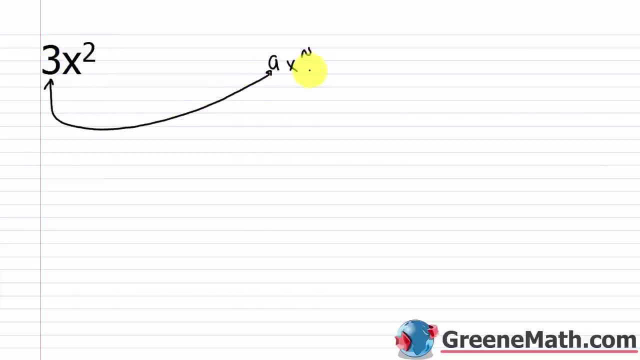 Then we have our variable x, and it's squared. Remember, n has to be a whole number. 2 is a whole number. So this is fine. This is a polynomial. This is a polynomial. So if somebody asked you on a test, is 3x squared a polynomial, you would say yes. But there's a further definition for this type of polynomial. If you have a polynomial, you would say yes. So if you have a polynomial, with a single term, meaning it's just one term here, 3x squared, it's called a monomial, okay? 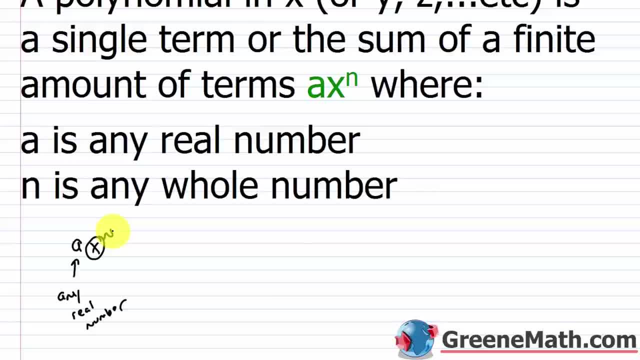 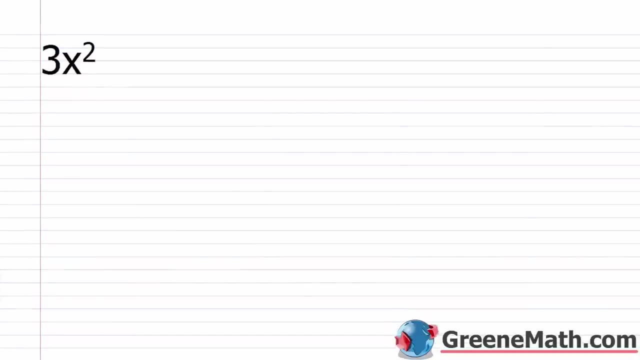 look for negatives And you want to look for fractions and things that are not whole numbers. If you see that in place here you don't have a polynomial, You don't have a polynomial, So this any whole number? So let me give you an example. We have something here: 3x squared, And remember. 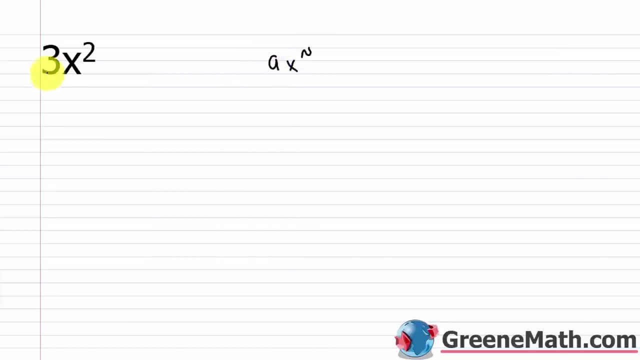 we're looking for ax to the power of n, So a can be any real number, And so 3 here is representing a, So that's fine. Then we have our variable x, and it's squared. Remember, n has to be a whole number. 2 is a whole number, So 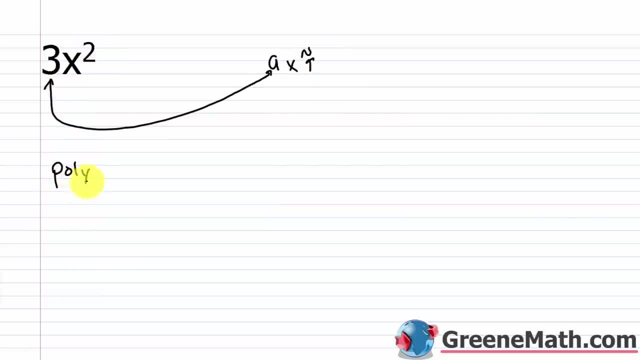 this is fine, This is a polynomial. This is a polynomial. So if somebody asked you on a test: is 3x squared a polynomial? you would say yes, But there's a further definition for this type of polynomial: If you have a polynomial with a single term, meaning it's just one term here. 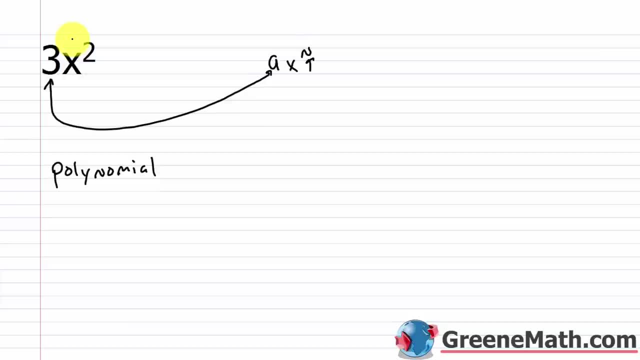 3x squared. it's called a monomial, So this has a special name: monomial. So let's say we saw something similar to this on a test. Let's say we saw something like 3x to the power of negative 2.. Would this be a polynomial? Well, the answer would be no. 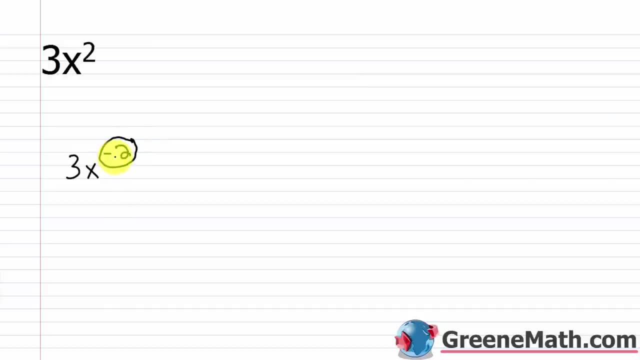 The exponent on x cannot be negative. It has to be a whole number. So 0,, 1,, 2,, 3, etc. etc. If you saw something like x raised to the power of 1, half, that's not a polynomial, That doesn't work. So we'd have 3x. 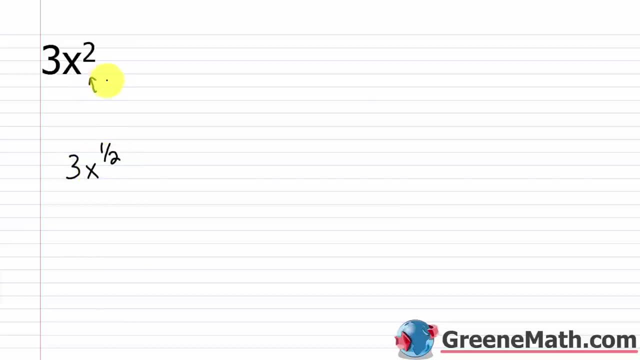 to the power of 1 half, not a polynomial. So this one, yes, This one, no. All right, what about this? 5x to the fourth power minus 7x squared. Just look at the variables and look at your exponents. So 5 is OK, Anything can be the coefficient for the variable. Remember. 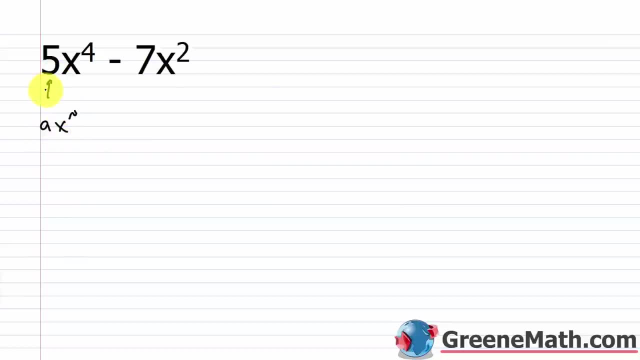 that's any real number, And we think about this as ax to the power of n, So this can be anything. The exponent on the variable has to be a whole number, And in this case it is. So this is OK. So this one checks out, And then this checks out as well: This is a 2.. 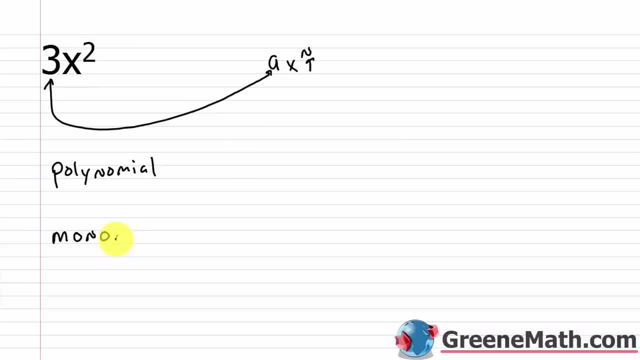 So this has a special name, monomial. So let's say we saw something similar to this on a test. Let's say we saw something like 3x to the power of negative 2. Would this be a polynomial? Well, 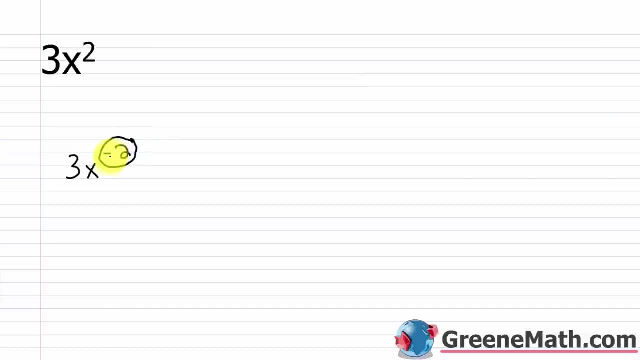 the answer would be no. The exponent on x cannot be negative. It has to be a whole number. So 0, 1, 2, 3, you know, et cetera, et cetera. If you saw something like x raised to the power of one 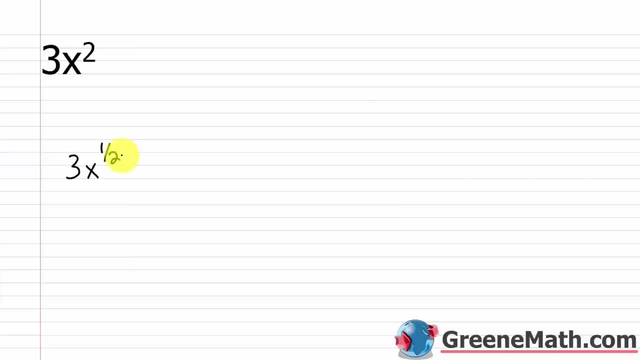 half, that's not a polynomial, okay? That doesn't work. So we'd have 3x to the power of one half, not a polynomial. So this one, yes. This one, no. All right, what about this? 5x to the fourth power 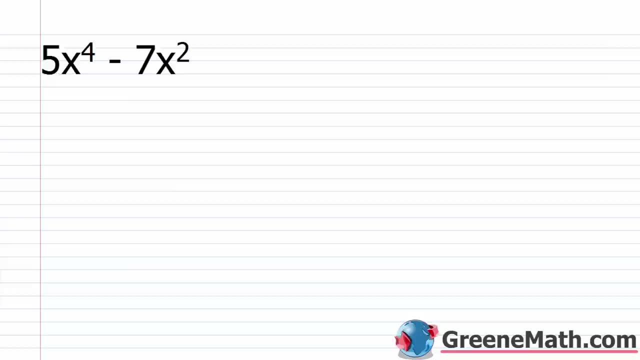 minus 7x squared. Just look at the variables and look at your exponents. So 5 is okay. Anything can be the coefficient for the variable. You can look at the variables and look at the exponents. 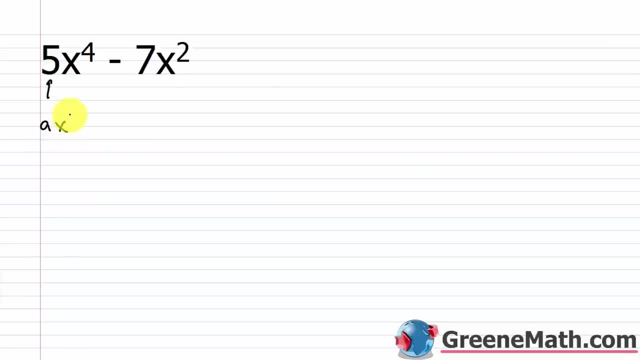 variable remember that's any real number and we think about this as ax to the power of n so this can be anything the exponent on the variable has to be a whole number and in this case it is so this is okay so this one checks out and then this checks out as well this is a 2 so you have a 4 and then a 2 so everything checks out so this is a polynomial now we have a special name for a polynomial with two terms only okay it's called a binomial okay so this is a polynomial with two terms only again a monomial which we saw in the previous example is a polynomial with one single term a binomial polynomial with two terms all right what about a variation of that so we have 5x to the power of negative 4 minus 7x squared well no this is not going to work if I have a polynomial with two terms I'm going to have a polynomial with two terms I look at my exponent on X it's a negative 4 you are not allowed to have a negative as an exponent when you're thinking about a polynomial right it's got to be a times X to the nth power where n is a whole number whole number this is an integer negative 4 so that's not going to work and later on we're 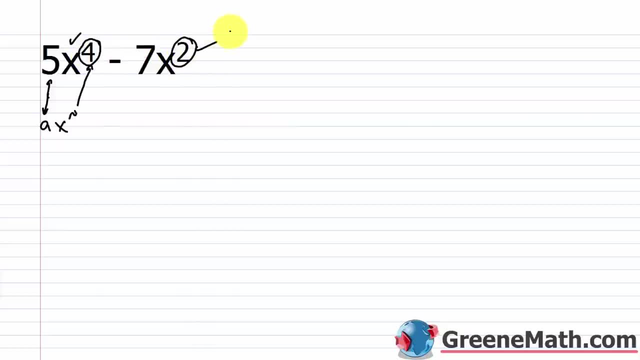 So you have a 4 and then a 2.. So everything checks out. So this is a polynomial. Now we have a special name for a polynomial with two terms only: It's called a binomial. OK, So this is a polynomial with two terms. 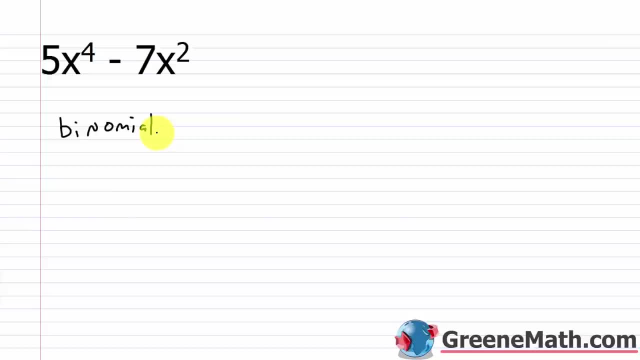 Only Again, a monomial, which we saw in the previous example, is a polynomial with one single term. A binomial polynomial with two terms. All right, what about a variation of that? So we have 5x to the power of negative, 4 minus 7x squared. Well, no, this is not going to work If I look at. 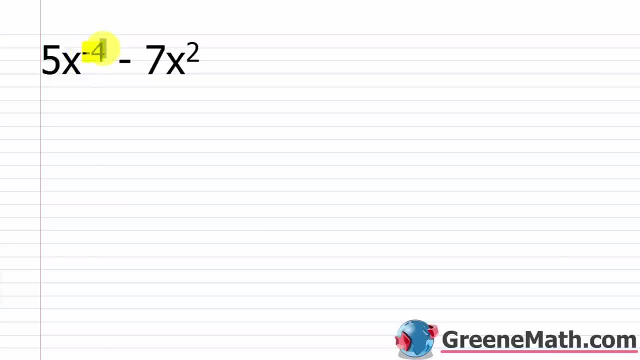 my exponent on x. it's a negative 4. You are not allowed to have a negative as an exponent when you're thinking about a polynomial. All right, it's got to be a times x to the nth power, where n is a whole number, Whole number. This is an integer. 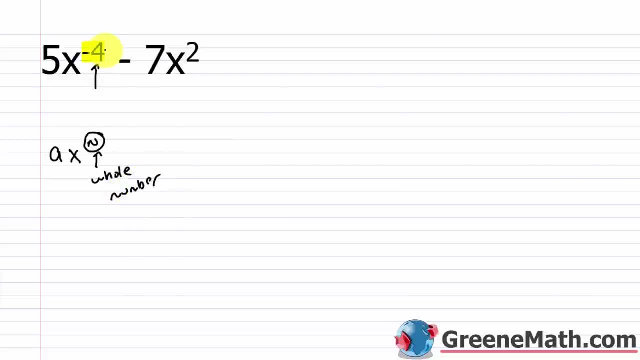 negative 4.. So that's not going to work And later on we're going to see that if you have something like this, really I could write this as what. I could write it as 5 over x to the 4th. 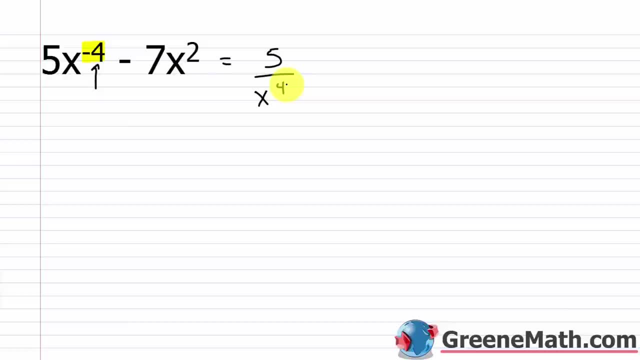 power right, using our rules for exponents that we've previously learned. then minus 7x squared, And we're going to talk about these types of expressions that are known as rational expressions. We'll see those here shortly, But for right now you just need. 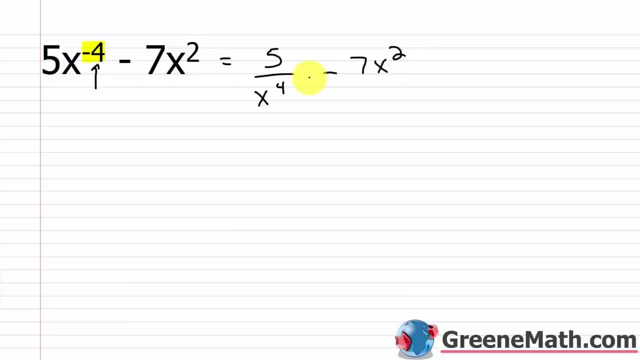 to know that when you see something like this, it's not a polynomial, All right, so you might also have polynomials that have more than one variable involved. Same rule is going to apply. You're basically looking at the variable parts and making sure that you don't have any. 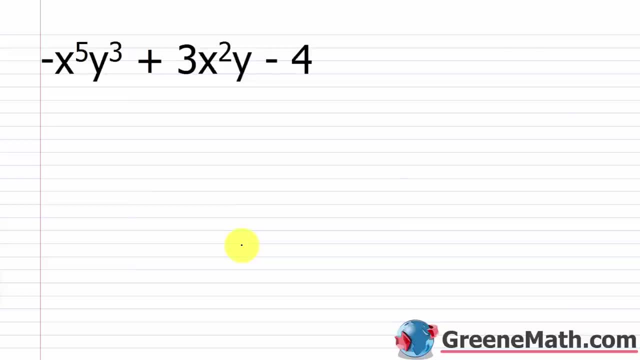 negative exponents and any fractional exponents. Basically you want the exponents to be whole numbers only. So if I look at negative x to the 5th power, y cubed plus 3x squared, y minus 4, just look at the exponents. So I have 5, a, 3, a, 2. This is really a phantom. 1 here. So 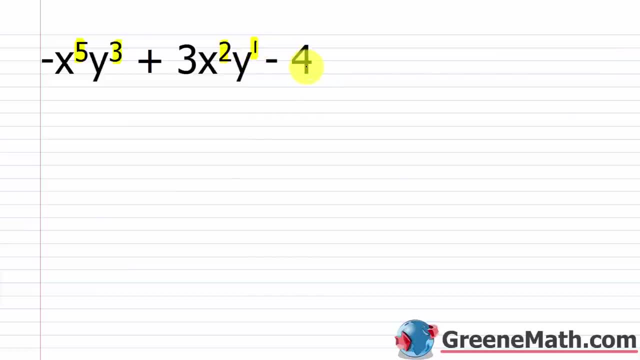 you can put that as a 1.. And then, if we wanted to, we could write this as 4 times x to the power of 0,, y to the power of 0. We could do that, Remember something to the power of 0 is 1.. So really. 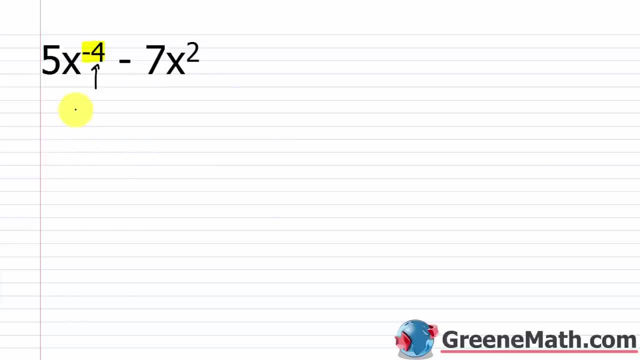 going to see that if you have something like this really I could write this as what I could write it as 5 over x to the fourth power right using our rules for exponents that we've previously learned then minus 7x squared and we're going to talk about these types of expressions they're known as rational expressions we'll see those here shortly but for right now you just need to know that when you see something like this it's not a polynomial all right so you might also have polynomials that have more than one variable involved same rule is going to apply you're basically looking at the variable parts and making sure that you don't have any negative exponents and any fractional exponents basically you want the exponents to be whole numbers only so if I look at negative X to the fifth power y cubed plus 3x squared y minus 4 just look at the exponent so I have 5 a 3 a 2 this is a really a phantom 1 here so you can put that as a 1 and then if we wanted to we could write this as 4 times X to the power of 0 Y to the power of 0 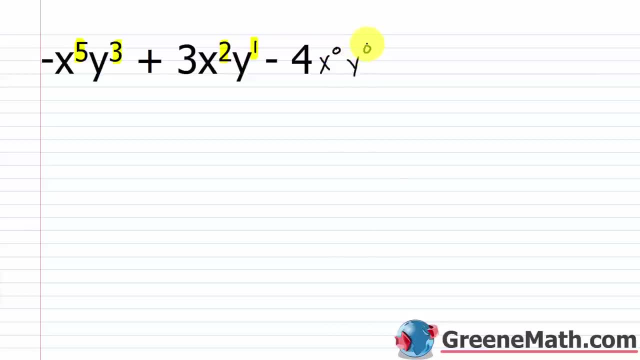 we could do that remember something to the power of 0 is 1 so really this would simplify to 4 times 1 but this doesn't violate our definition of a polynomial because the exponents for the variables have to be whole numbers 0 is a whole number so this would still be a polynomial so we have negative X to the fifth power y cubed plus 3x squared y minus 4 this is a polynomial now if I see 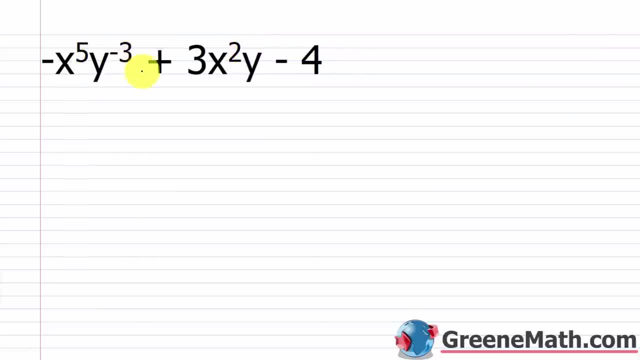 something like negative X to the fifth power Y to the power of negative 3 plus 3x squared y minus 4 the difference here is that I have a negative 3 and so now because I don't have a whole number as my exponent this 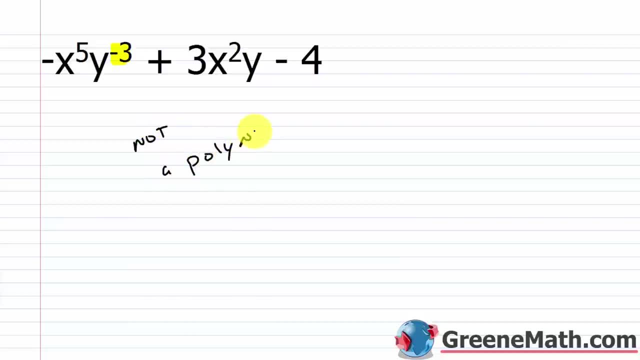 is not a polynomial and again you might see a variation of this you might see something like negative X to the fifth power let's say Y to the power of 1 3rd plus 3 X to the 1 half power Y minus 4 you can't have fractional exponents either again everything has to be 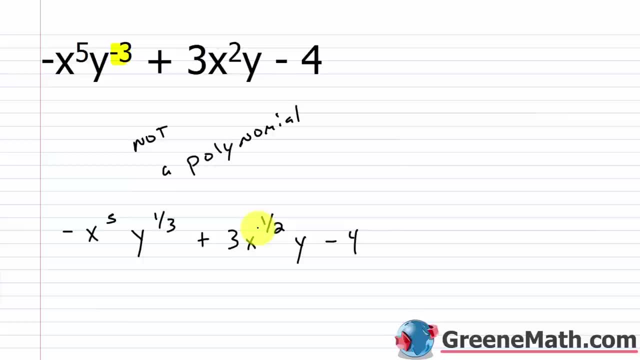 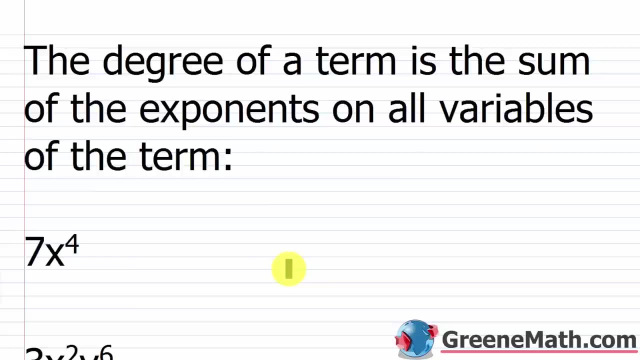 number in terms of the exponent for you to have a polynomial. All right so kind of the next thing we want to talk about is the degree of a term. Okay so you're going to have a degree for your term and then you're going to have a degree of the polynomial. Okay they could be the same or 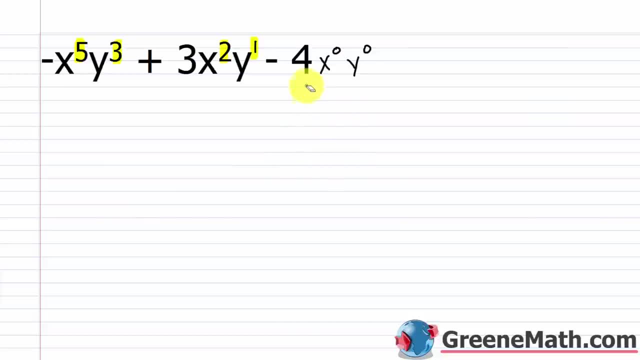 this would simplify to 4 times 1.. But this doesn't violate our definition of a polynomial, because the exponents for the variables have to be whole numbers. 0 is a whole number, so this would still be a polynomial. So we have negative x to the 5th power, y cubed plus 3x squared, y minus 4.. This 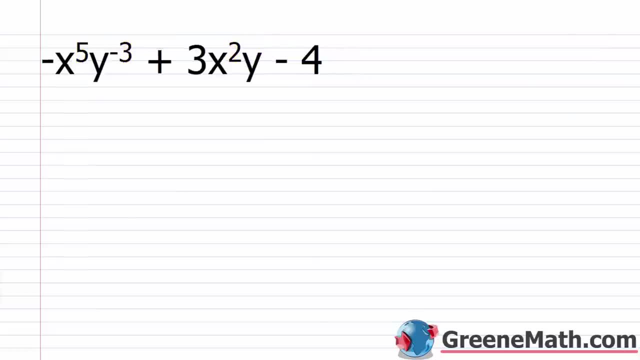 is a polynomial. Now, if I see something like negative x to the 5th power, y to the power of negative, 3 plus 3x squared y minus 4, the difference here is that I have a negative 3.. 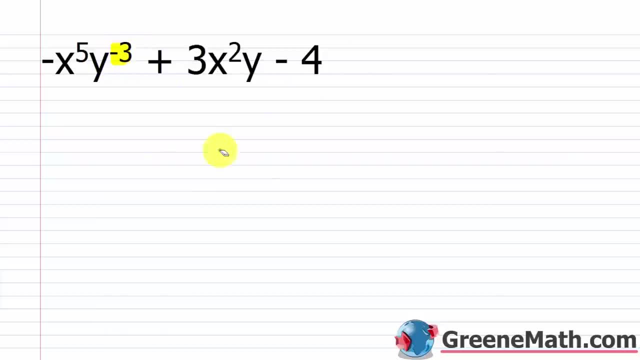 And so now, because I don't have a whole number as my exponent, this is not a polynomial, And again you might see a variation of this. You might see something like negative x to the 5th power, let's say y to the power of 1 3rd plus 3x to the 1 half power, y minus 4.. 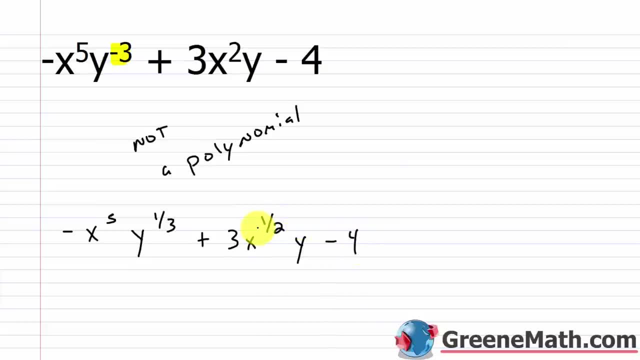 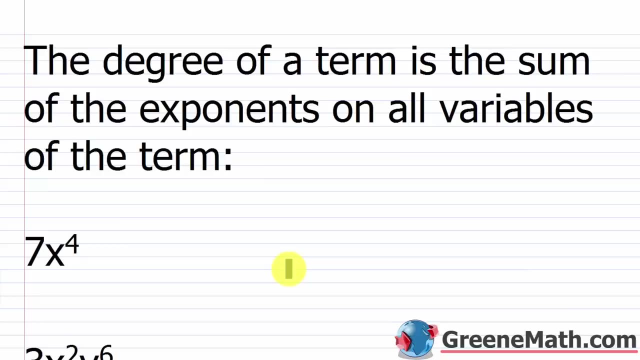 You can't have fractional exponents either. Again, everything has to be a whole number in terms of the exponent for you to have a polynomial. All right, so kind of. the next thing we want to talk about is the degree of a term, So you're going to have a degree for your. 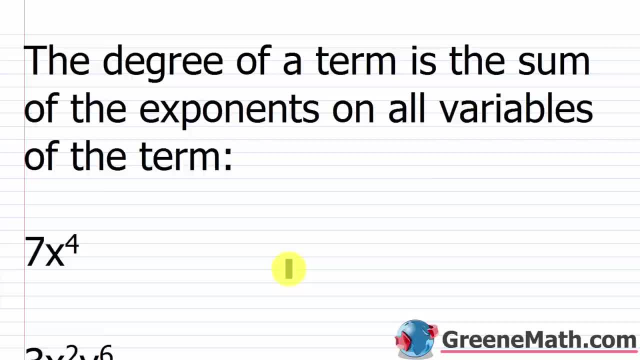 term have a degree of the polynomial. They could be the same or they could be different. It just depends on the situation. So the degree of a term is the sum of the exponents on all variables of the term. So, for example, if I want to look at 7x to the fourth power, what's the degree of this? 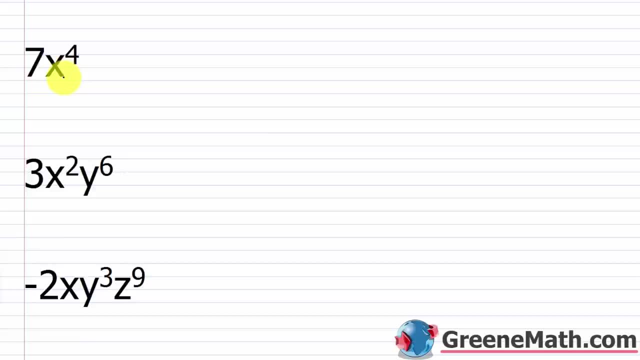 term. Well, if I look at the definition again, the degree of the term is the sum of all exponents on all variables of the term. So I just have an exponent of 4 here and that's it. So the degree. 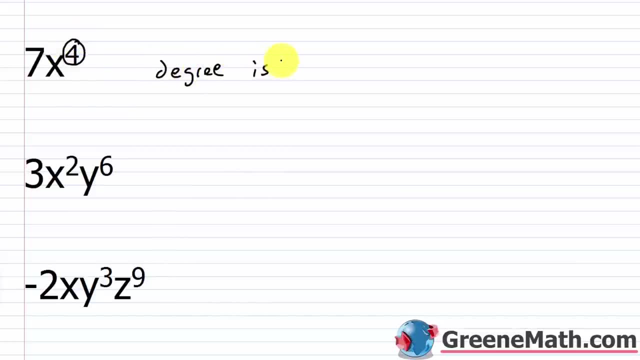 is 4, and that's for the term. It's also the degree of the polynomial, but again, those could be different. It just depends on the situation. So the degree- let me be more specific and say the degree of the term. 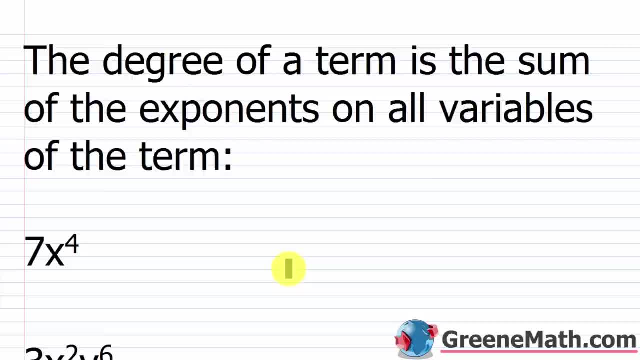 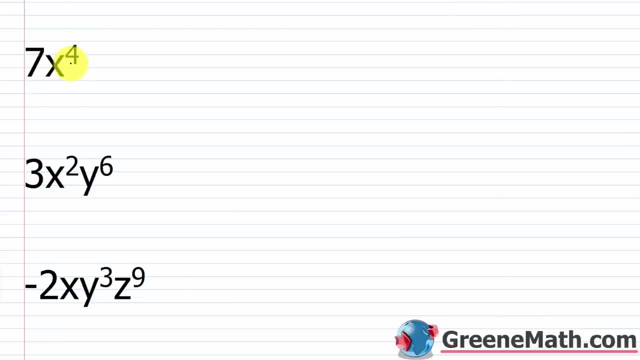 they could be different just depends on the situation. So the degree of a term okay the degree of a term is the sum of the exponents on all variables of the term. So for example if I want to look at seven X to the fourth power what's the degree of this term? Well if I look at the definition again the degree of the term is the sum of all exponents on all variables of the term. So I just have an exponent of four here and that's it. So the degree is four and that's for the term. It's also the degree of the polynomial but again those could be different it just depends on the situation. So the degree let me be more specific and say the degree. 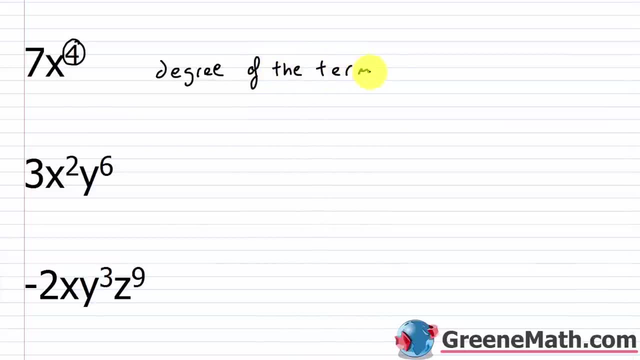 of the term is 4. Now for this one, we have 3x squared y to the sixth power. 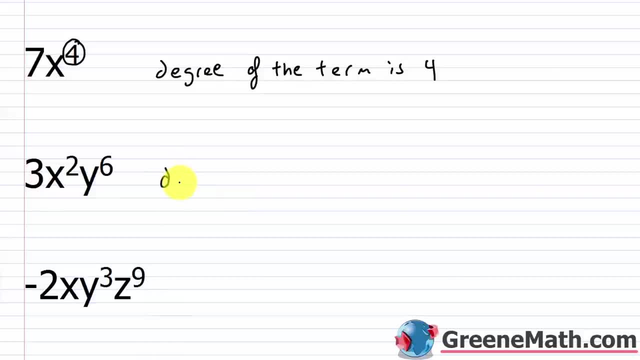 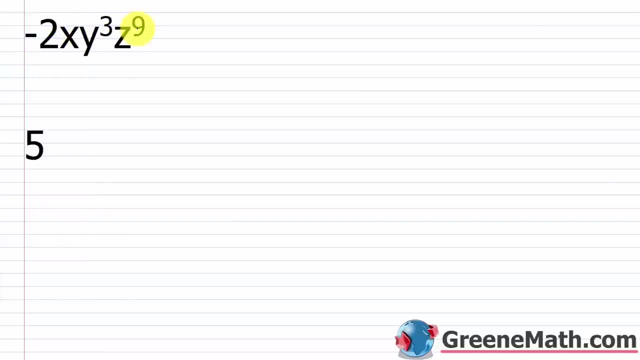 So the degree here is going to be 8. The degree of the term is 8. And that's because I looked at the exponent here, that's 2. And I looked at the exponent here, that's 6. I just summed them. 2 plus 6 is 8. So that's how I got them. So if I look at the next one, I have a negative 2xy cubed z to the ninth. Again, I'm just going to sum my exponents. Now a common mistake here, you don't see anything written as an exponent for x. But remember, it's a 1. x to the first power is x. So don't forget that because a lot of students will just go, okay, 3 plus 9 is 12. And they're done. They forget about that x raised to the, the first power. So you really have a 1 here, a 3 here and a 9 here. So 1 plus 3 is 4. 4 plus 9 is 13. So the degree, the degree of the term is 13. And what if I see a single number like 5? 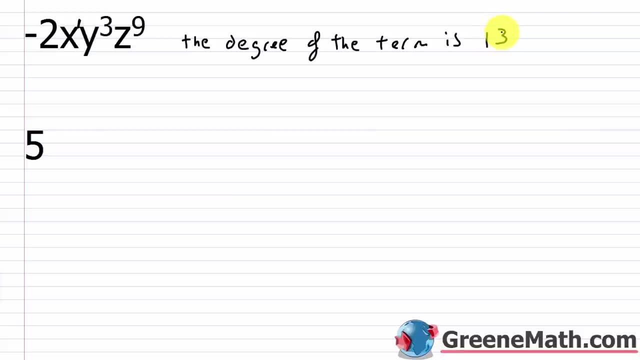 And someone asks you, what's the degree of this term? Well, remember, as I just showed you, you could write this as 5 times some variable raised to the power of 0. 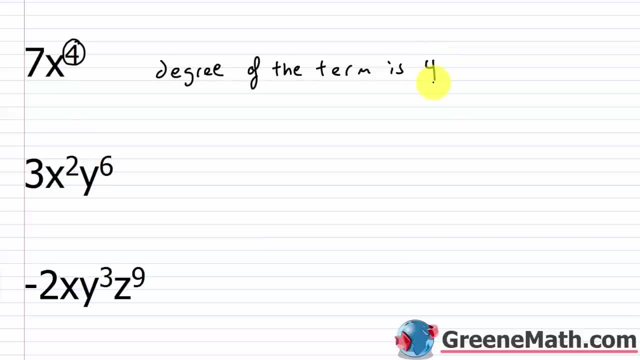 is 4.. Now for this one, we have 3x squared y to the sixth power, So the degree here is going to be 8.. The degree of the term is 8.. And that's because I looked at the exponent here, that's 2, and I looked at the exponent here, that's 6.. I just summed them: 2 plus. 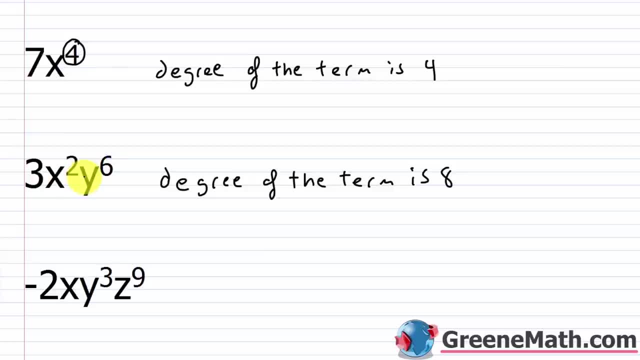 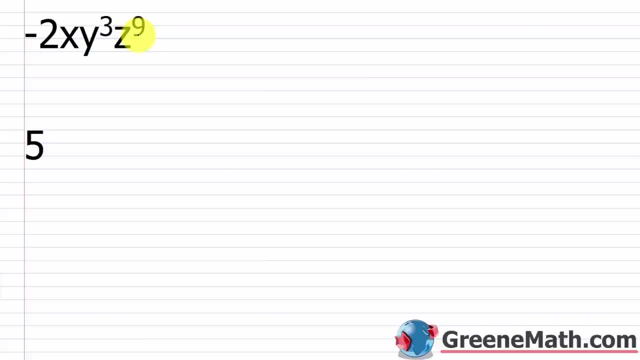 6 is 8.. So that's how I got them. So if I look at the next one, I have negative 2xy, cubed z to the ninth. Again. I'm just going to sum my exponents Now. a common mistake here. you don't see anything. 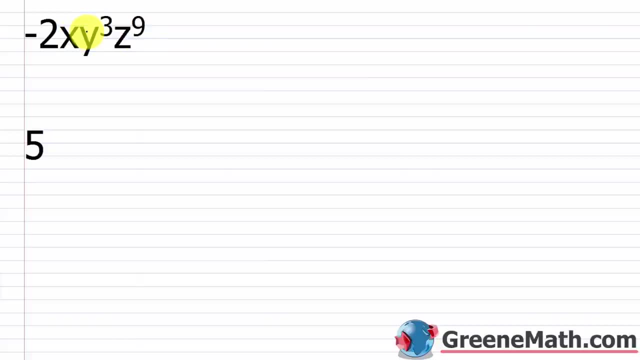 written as an exponent for x, But remember it's a 1. x to the first power is x, So don't forget that because a lot of students will just go: okay, 3 plus 9 is 12, and they're done. They forget about. 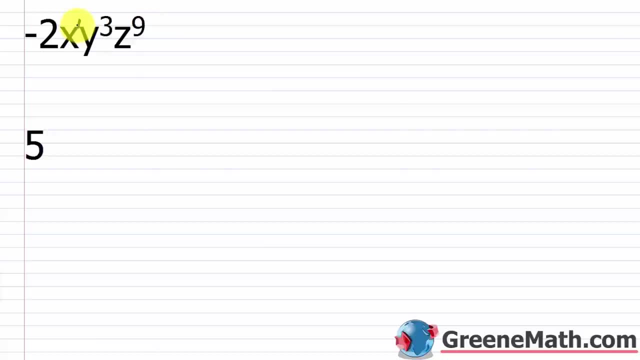 that x raised to the first power. So you really have a 1 here, a 3 here and a 9 here. So 1 plus 3 is 4.. 4 plus 9 is 13.. So the degree, the degree of the term. 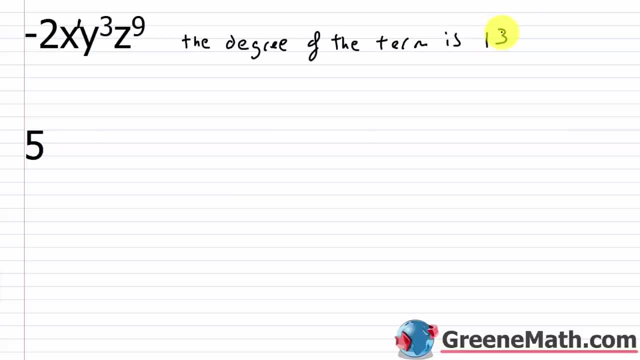 is 13.. And what if I see a single number like 5, and someone asks you what's the degree of this term? Well, remember, as I just showed you, you could write this as 5 times some variable raised to the power of 0. So if I sum the exponents here, I just have an exponent of 0, and that's. 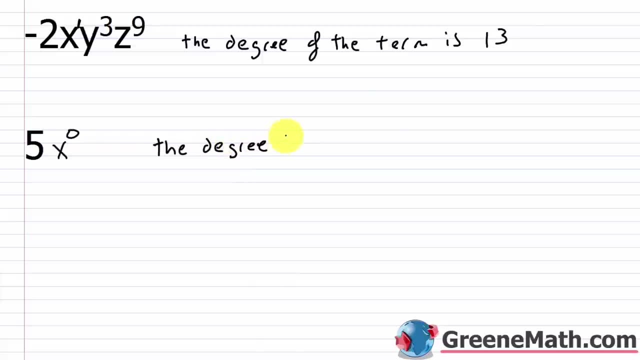 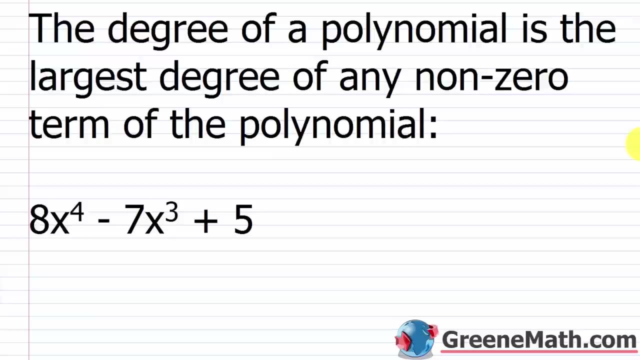 my degree. So the degree of the term is 0.. So now let's talk about the degree of a polynomial. So the degree of a polynomial is the largest degree of any non-zero term of the polynomial. So essentially what you're going to do, 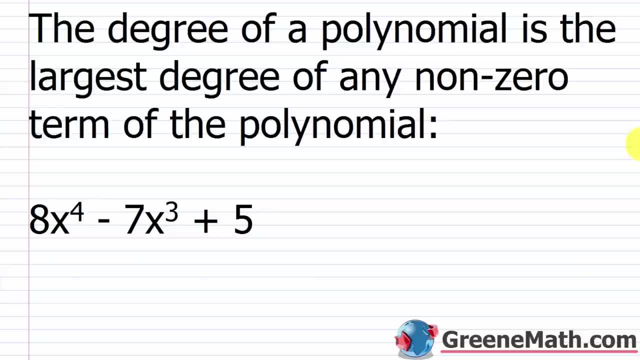 is: look at each term of the polynomial, find out which one has the largest degree, and then that's the degree of the polynomial. So, for example, if we have 8x to the fourth power, minus 7x, cubed plus 5, I look here I have a degree of 4, a degree of 3, and then a degree of basically 0. I could put. 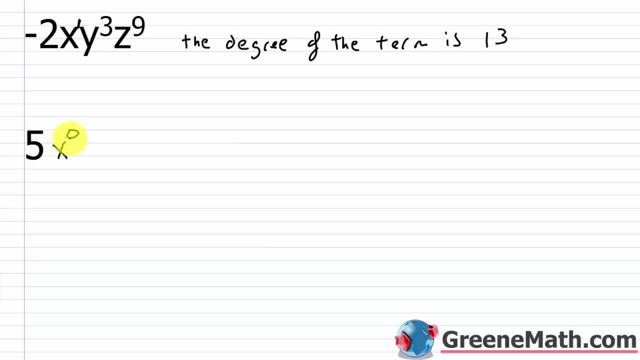 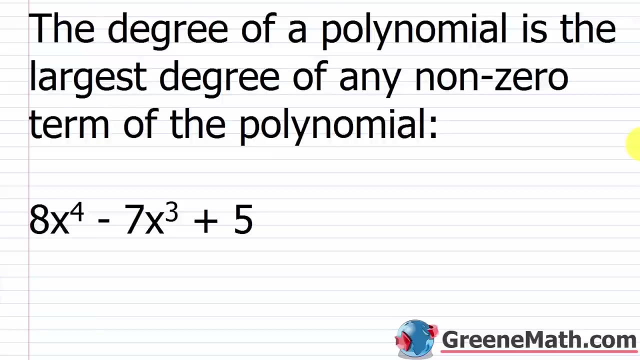 So if I sum the exponents here, I just have an exponent of 0. And that's my degree. So the degree of the term is 0. All right, so now let's talk about the degree of a polynomial. So the degree of a polynomial is the largest degree of any non-zero term of the polynomial. So essentially, what you're going to do is look at each term of the polynomial, 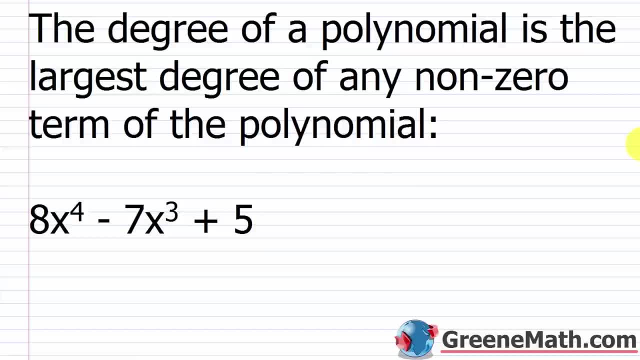 find out which one has the largest degree, and then that's the degree of the polynomial. So for example, if we have 8x to the fourth power minus 7x cubed plus 5, I look here, I have a degree of 4, a degree of 3, and then a degree of basically 0, right? I could put this as x to the power of 0. So I know that the largest degree 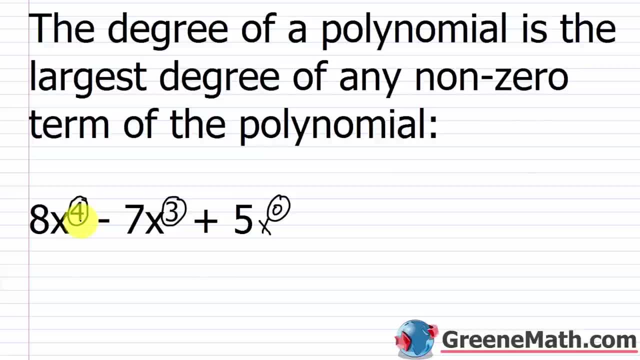 of any term is 4. So the degree of the polynomial is 4. So this polynomial 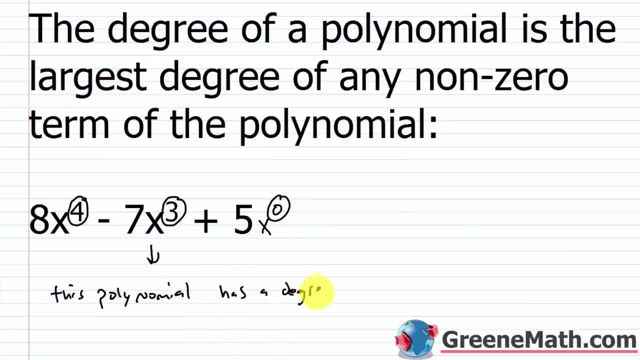 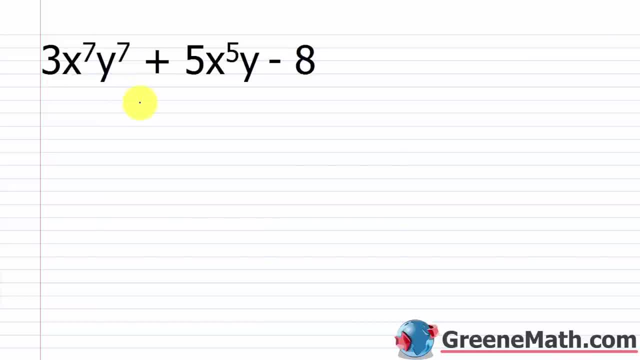 has a degree of 4. Well, again, when you start getting stuff with more than one variable in it, and you're going to get a lot of that in algebra 2, not so much in algebra 1, you really have to take your time and add all of them up and try to see what the largest degree is for any term. Sometimes you'll get like 7 or 8 of these in a row. They're trying to trip you up, and you'll have multiple, multiple 1s in each one. So you really have to go through and take your time. 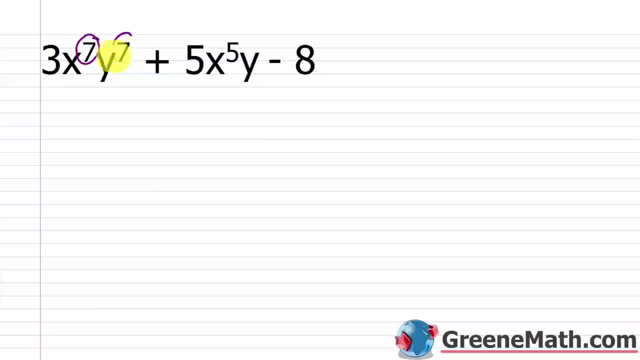 So for this one, I just count the exponents. So I have a 7 and a 7. So 7 plus 7 is 14. So my degree for this term is 14. For this one, I have a 5, and remember, I have a 1. So you have to remember that. So important that you don't forget. So this is a 1 there. So 5 plus 1 is 6. And then here, if I see a constant, the degree is always going to be 0, right? Because I could write this as x to the power of 0. So I don't really need to put that the degree of 0. Obviously, 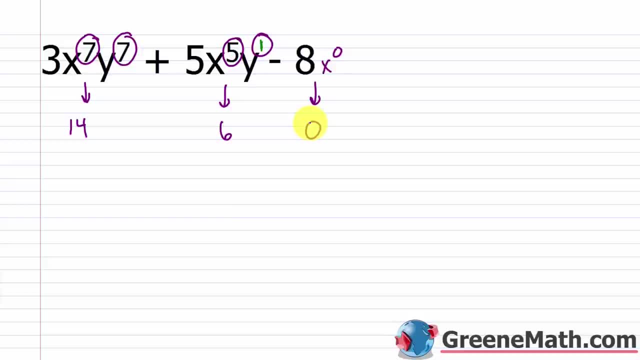 that's not going to be the worst. So I'm going to put that as x to the power of 0. Unless I just had, you know, a single term polynomial that was just a constant. 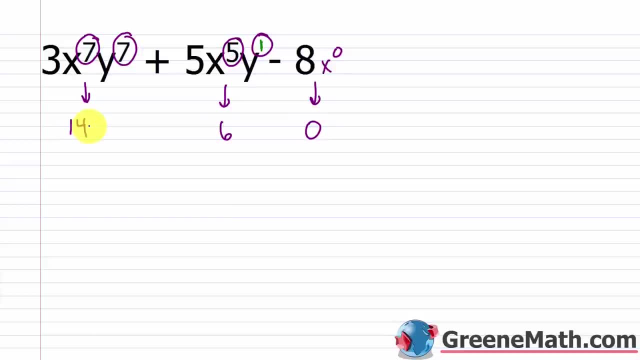 So in this case, 14 is the largest degree of any term. So the degree for the polynomial here is 14. 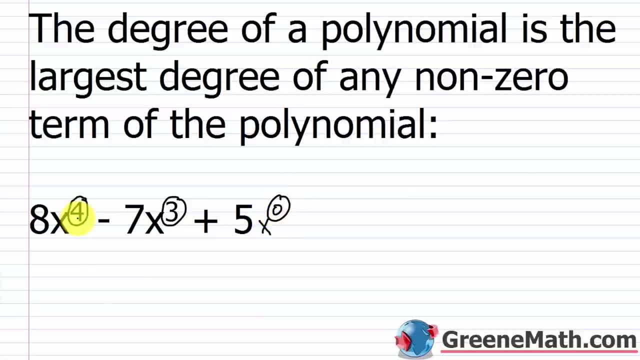 4 to the power of 0. So I know that the largest degree of any term is 4, so the degree of the polynomial is 4.. So this polynomial has a degree of 4.. Well, again, when you start getting stuff, 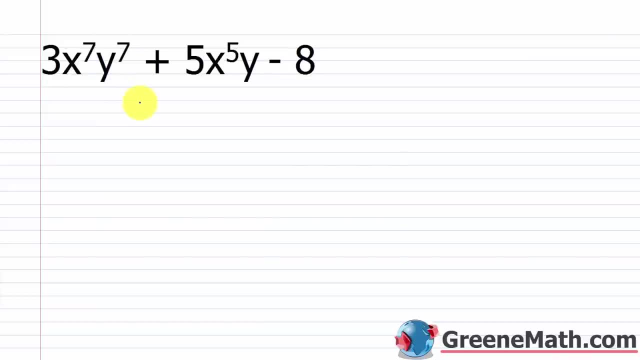 with more than one variable in it, and you're going to get a lot of that in Algebra 2,, not so much in Algebra 1, you really have to take your time and add all of these things together. So for this one I just count the exponents. So I have a 7 and a 7.. So 7 plus 7 is 14.. So my degree. 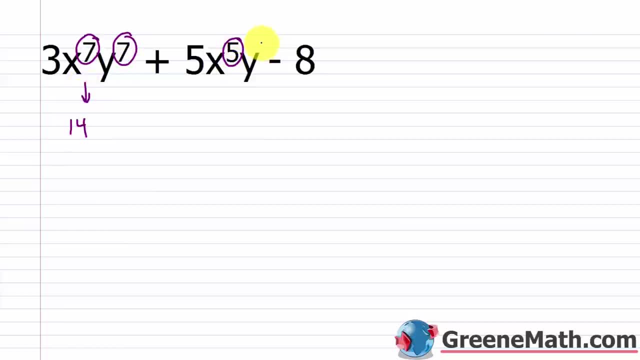 for this term is 14.. For this one I have a 5, and remember I have a 1.. So you have to remember that So important that you don't forget. So for this one I have a 5, and remember I have a 1.. 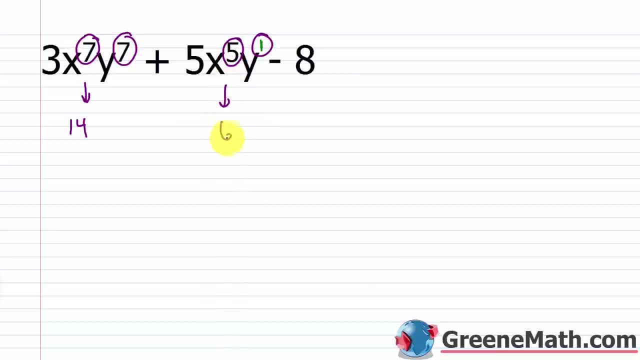 So this is a 1 there. So 5 plus 1 is 6.. And then here, if I see a constant, the degree is always going to be 0, because I could write this as x to the power of 0. So I don't really need to put. 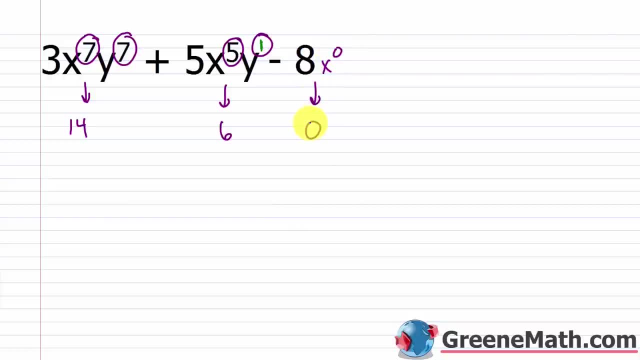 that the degree of 0. Obviously that's not going to be the winner. unless I just had a single term polynomial, that was just a constant. So in this case, 14 is the largest degree of any term. So the degree for the polynomial here is 14.. So this polynomial 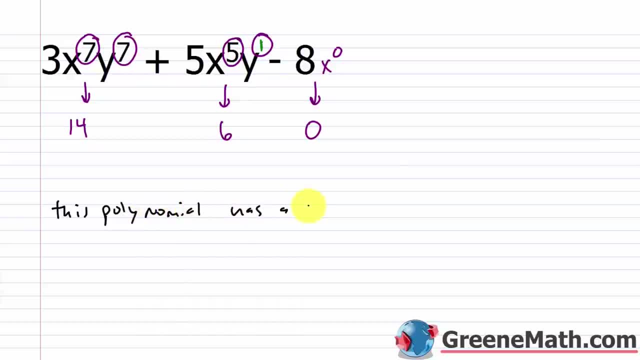 as a degree of 14.. So what about something like a constant, like negative 10?? Well, the first thing is: how do we make this match the definition of a polynomial? Remember a polynomial? you get something like ax to the power of n, where a is a real number and n is a whole number. We could 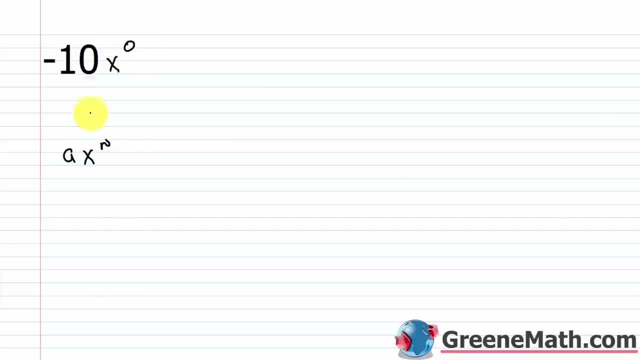 write negative 10 times again x to the power of 0. And this fits your definition. a is a real number, That's negative 10 times x to the power of 0. And this fits your definition. So you could. 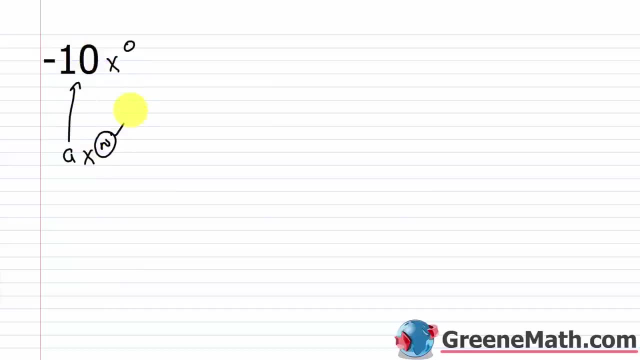 write negative 10, x is there, and then n has to be a whole number, 0 is a whole number, And then, if we were to simplify this, it's just negative 10 times 1, which is what? It's, just negative 10.. 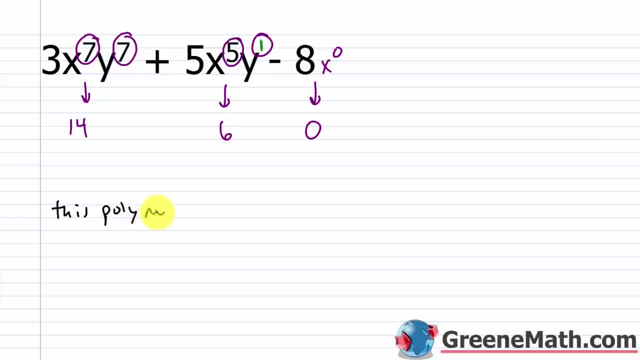 So this polynomial has a degree of 14. So what about something like a constant like negative 10? 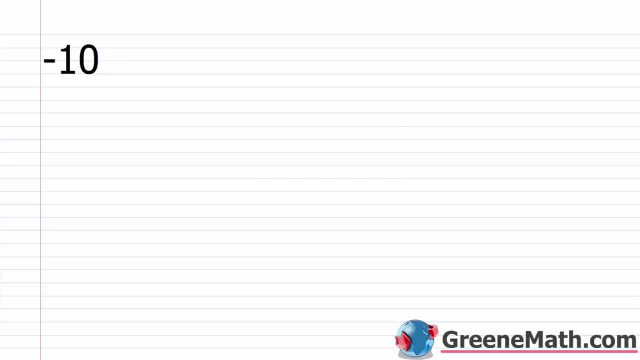 Well, the first thing is, how do we make this match the definition of a polynomial? Remember, a polynomial, you get something like ax to the power of n, where a is a real number, and n is a whole number. We could write negative 10 times, again, x to the power of 0. And this fits your definition. a is a real number. That's negative 10. x is there. And then n has to be a 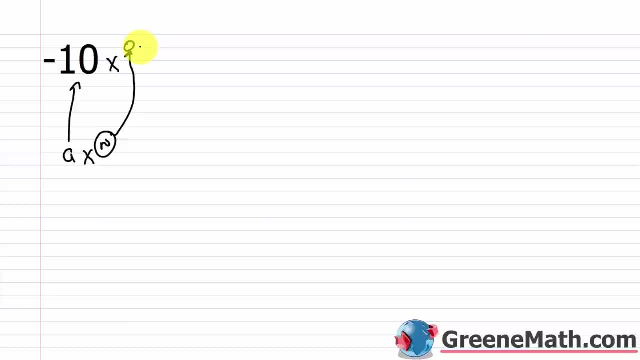 whole number. 0 is a whole number. And then if we were to simplify this, it's just negative 10 times 1, which is what? It's just negative 10, right? So that matches up with our definition. 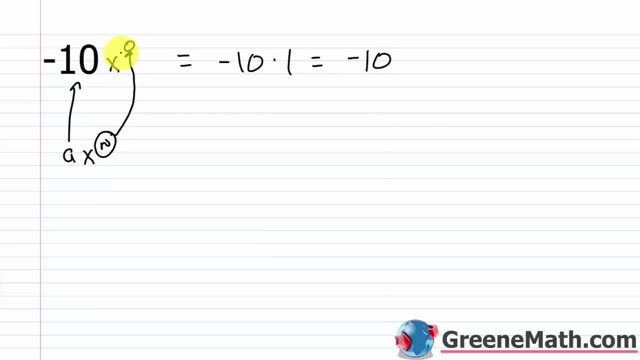 Now, for the degree for this thing, again, you're just looking at the exponent, which in this case is 0. So the polynomial here just has a degree of 0. So this polynomial has a degree of 0. So just look out for that on a test, because you might see a single number like 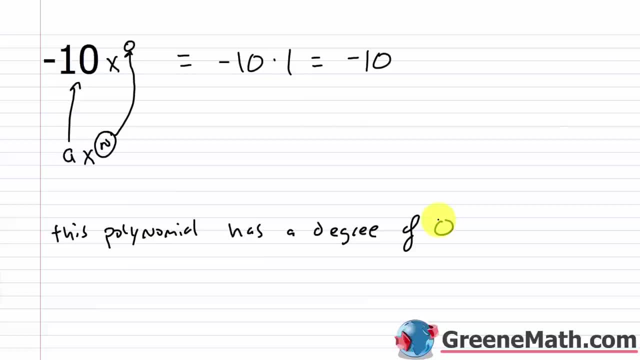 that and say, well, this doesn't have a degree. There's no variable to look at. Yes, it does. It doesn't have a degree. It doesn't have a number. It doesn't have a number. It doesn't have a Variable is whatever you want it to be. It could be x or y or z or whatever you choose. 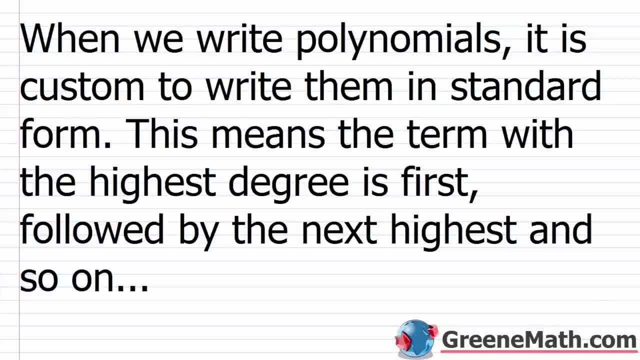 Raised to the power of 0. Alright, so kind of the last thing we're going to talk about before we get into actually adding and subtracting polynomials. 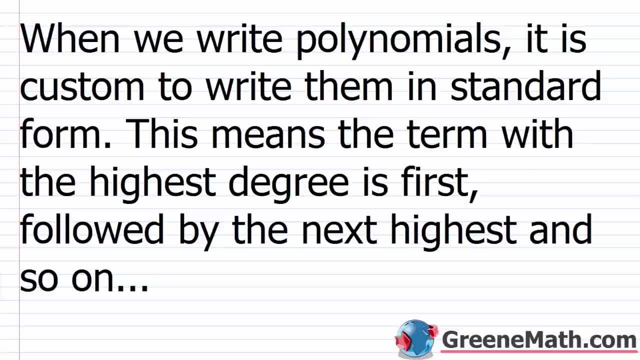 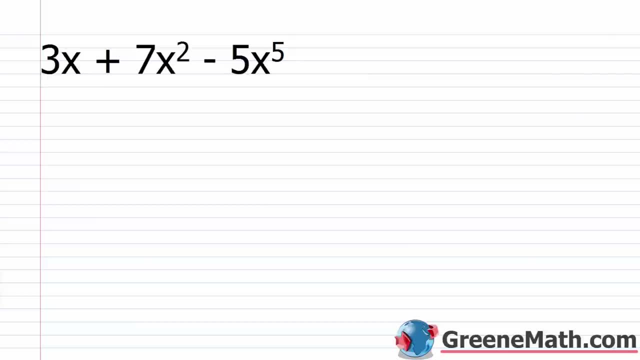 When we write polynomials, it is custom to write them in what's known as standard form. So this means the term with the highest degree is first, then followed by the next highest, and so on and so forth. So something like this, 3x plus 7x squared minus 5x to the 5th. So the term with the highest degree would be this one, negative 5x to the 5th power. Your exponent there is 5, this is 2, and this is basically 1. So this would be first, so you'd have negative 5x to the 5th power. The next highest, you have a 2 here and you have a 1 here. So this is the next highest, so 7x squared, and then this is the last term, so plus 3x. So this is that polynomial written in standard form. 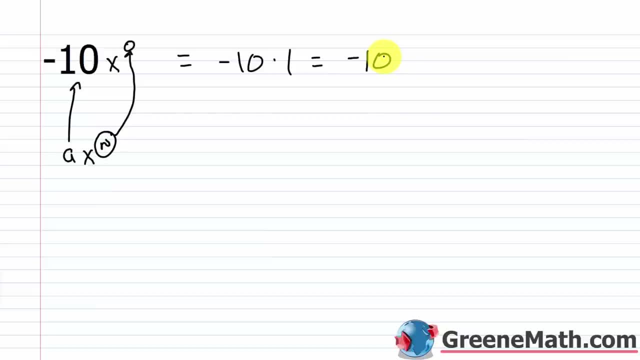 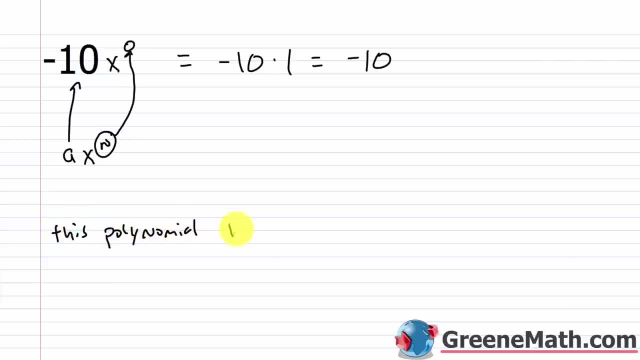 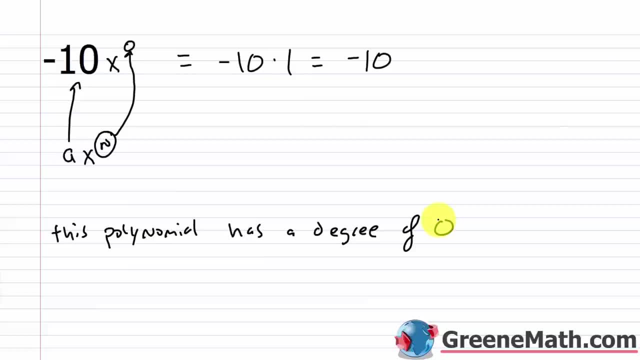 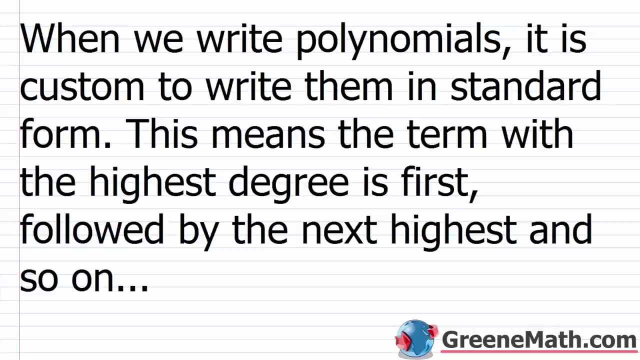 well, this doesn't have a degree. There's no variable to look at. Yes, it does. The variable is whatever you want it to be. It could be x or y or z or whatever you choose, raised to the power of 0.. All right, so kind of the last thing we're going to talk about before we get into actually. 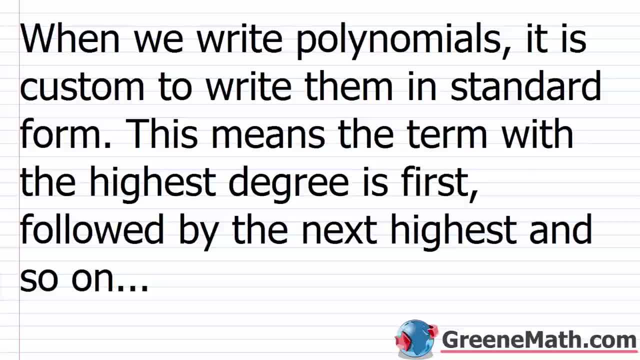 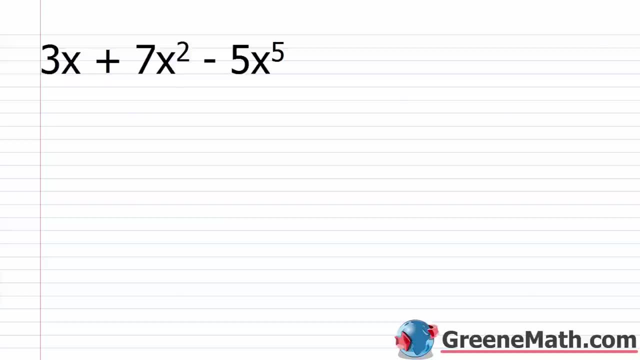 adding and subtracting polynomials. When we write polynomials, it is custom to write them in what's known as standard form. So this means the term with the highest degree is first, then followed by the next highest, and so on and so forth. So something like this: 3x plus 7x, squared minus 5x. 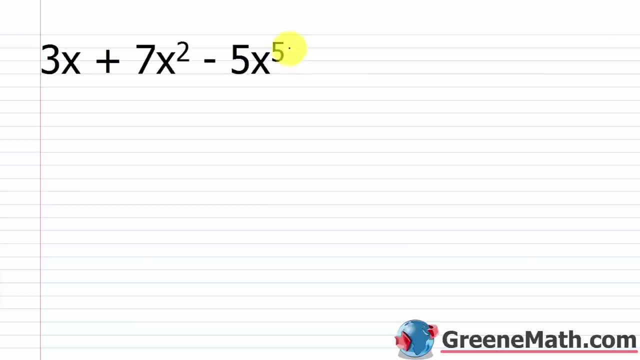 to the fifth. So the term with the highest degree would be this: one negative 5x to the fifth power. right, your exponent. there is five, this is two and this is basically one. So this would be first, so you'd have negative 5x to the fifth power, the next highest. you have a two here and you have a. 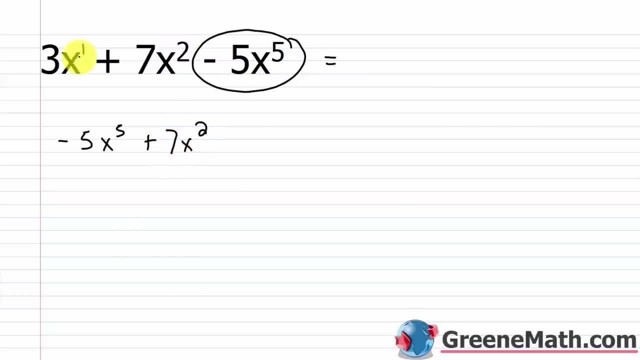 one here. So this is the next highest, so 7x squared, and then this is the last term, so plus 3x. So this is that polynomial written in standard form. Again, it's just placing it where the term with the highest degree or the largest degree is first, then followed by the next largest, and so on. 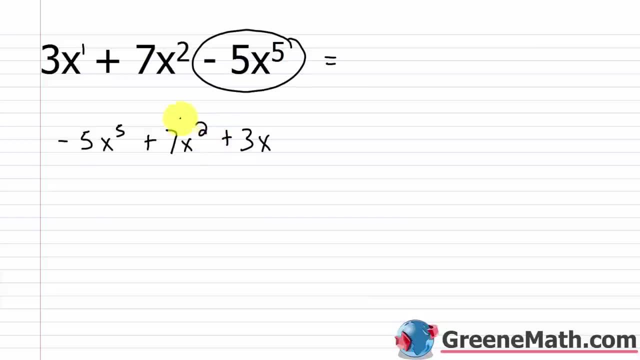 and so forth. So we have: this term has a degree of five, then we have the next highest degree, and so on and so forth. So this term has a degree of five, then this term has a degree of two, then this term has a degree of one right, so on and so forth. 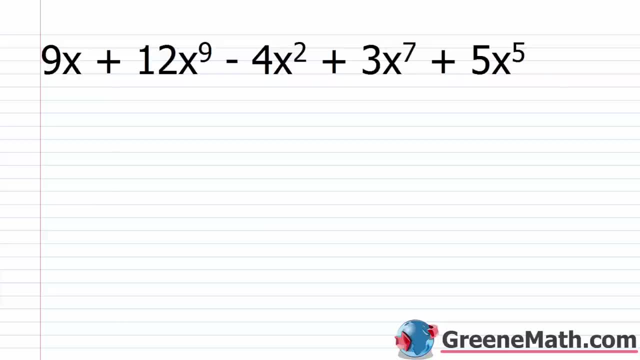 All right, let's take a look at one more of these. So we have 9x plus 12x to the ninth power, minus 4x squared, plus 3x to the seventh power, plus 5x to the fifth power, So the highest degree is going. 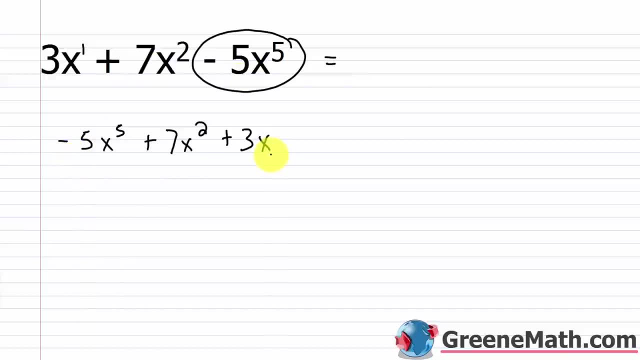 Again, it's just placing it where the term with the highest degree, or the largest degree, is first, then followed by the next largest, and so on and so forth. 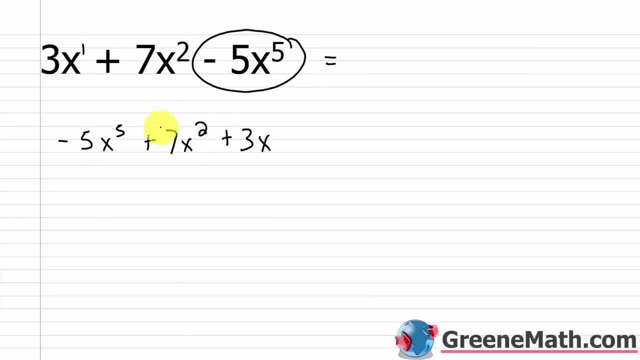 So we have this term has a degree of 5, then this term has a degree of 2, then this term has a degree of 1. Alright, so on and so forth. Alright, let's take a look at one more of these. 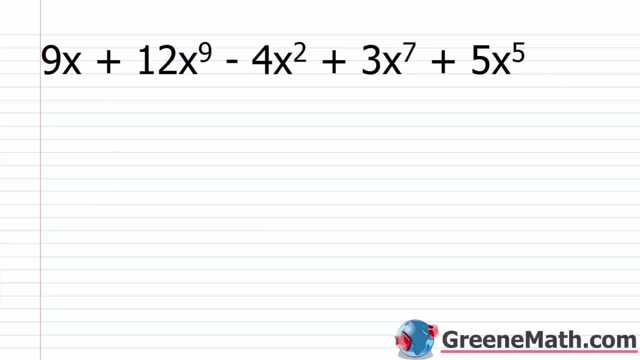 So we have 9x plus 12x to the 9th power minus 4x squared plus 3x to the 7th power plus 5x to the 5th power. So the highest degree is going to go first. So if I look here, 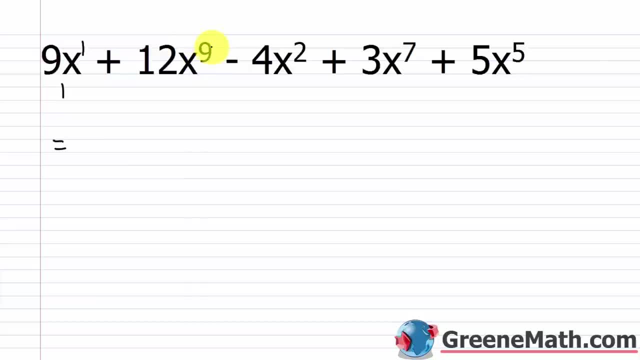 I have a degree of 1, I have a degree of 9, I have a degree of 2, a degree of 7, and a degree of 5. 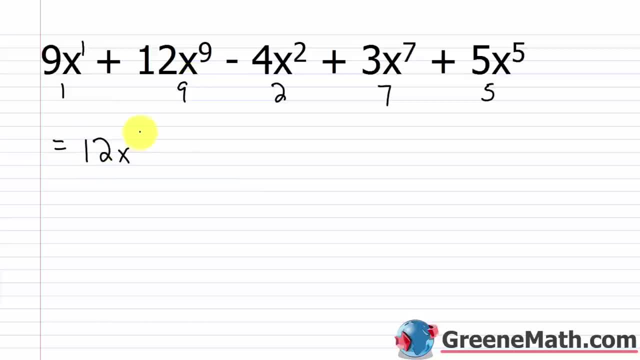 So 9 is the largest, so I'd start by writing 12x to the 9th power. And I'm just going to line this out just so I know I've used it already. 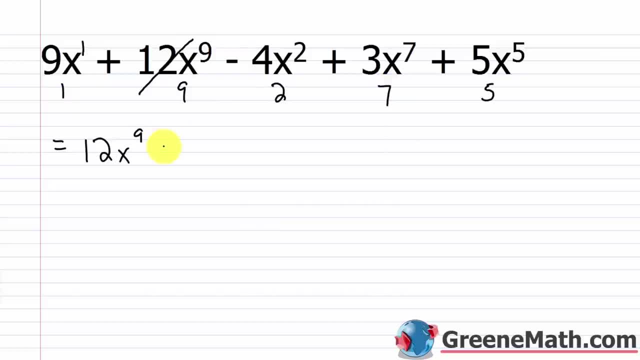 And if I look at the numbers that are remaining, 7 is the next largest, so then plus 3x to the 7th power. Line that out. Then 5 is the next largest, so plus 5x to the 5th power. Line that out. Then I have this negative 4x squared, right, that 2 is the next largest, so minus 4x squared. Line that out, and then this is what's left, so plus 9x. So I can just erase all this now. 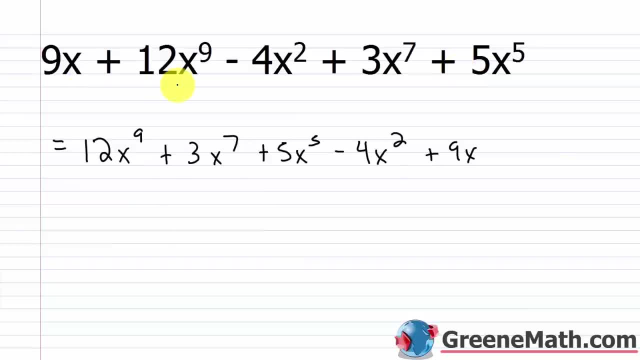 And so 9x plus 12x to the 9th power minus 4x squared plus 3x to the 7th power plus 5x to the 5th power, written in standard form, is going to be equal to 12x to the 9th power, that's first, plus 3x to the 7th power, that's second. 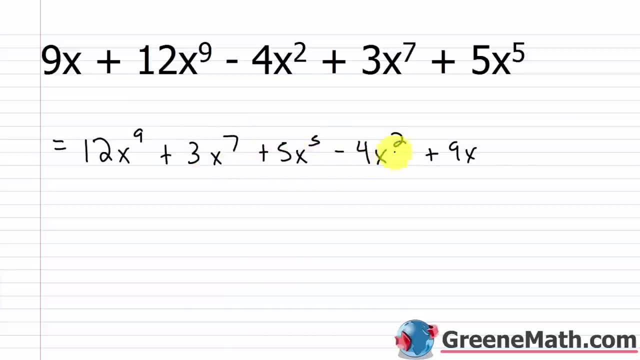 Plus 5x to the 5th power, that's third, minus 4x squared, that's fourth, and then finally, in 5th place, plus 9x. So you can see how it goes in descending order. 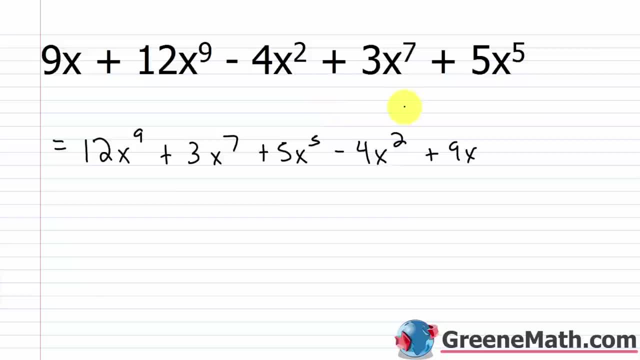 You have an x to the 9th, an x to the 7th, an x to the 5th, an x squared, and then an x, or an x to the 1st power. 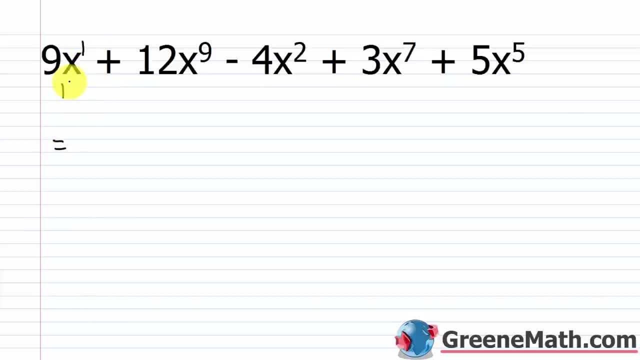 to go first. So if I look here, I have a degree of one, I have a degree of nine, I have a degree of two, a degree of seven and a degree of five. So nine is the largest. so I'd start by writing 12x. 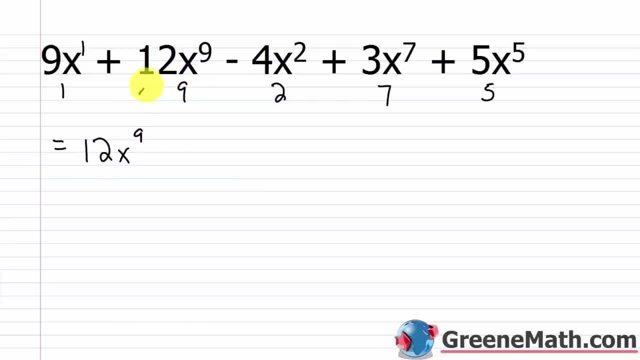 to the ninth power- and I'm just going to line this out just so I know I've used it already- And if I look at the numbers that are remaining, seven is the next largest, so then plus 3x to the seventh power. line that out. then five is the next largest, so plus 5x to the fifth power. 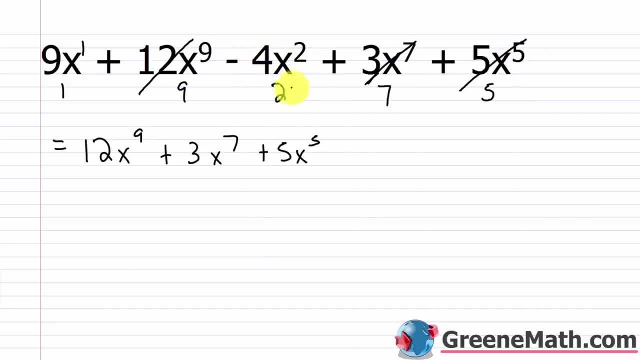 line that out. then I have this negative 4x squared right. that two is the next largest, so minus 4x squared line that out. and then this is what's left: so plus 9x. So I can just erase all this now. and so 9x plus 12x to the ninth power, minus 4x squared plus 3x to. 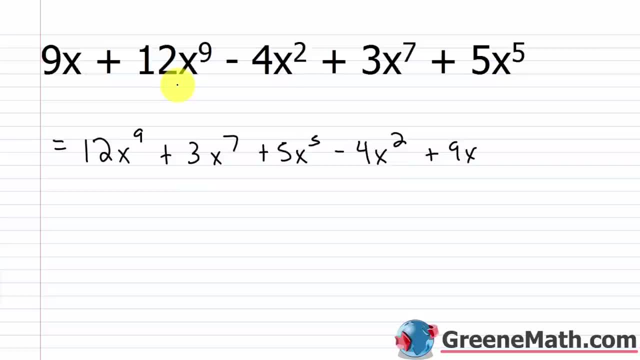 the seventh power plus 5x to the fifth power. written in standard form is going to be equal to 12x to the ninth power. that's first plus 3x. to the seventh power, that's second plus 5x. to the fifth power. that's third minus 4x. squared, that's fourth, and then finally, in fifth place, plus 9x. 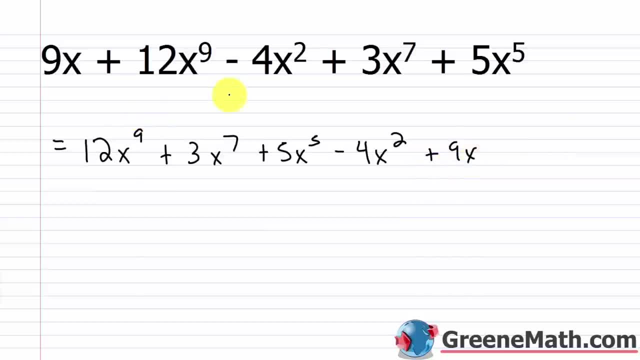 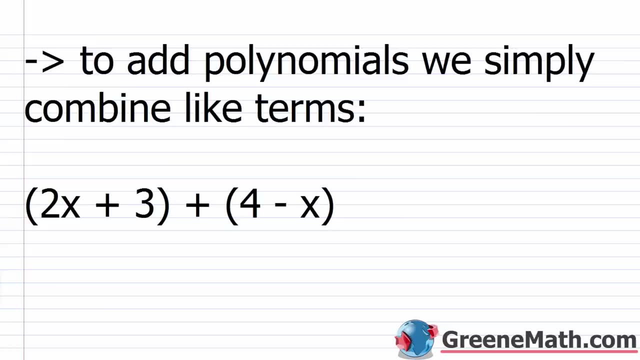 So you can see how it goes in descending order. You have an x to the ninth, an x to the seventh, an x to the fifth, an x squared, and then an x or an x to the first power. Alright, so now let's get to the meat of the lesson, and this is actually the easiest part. 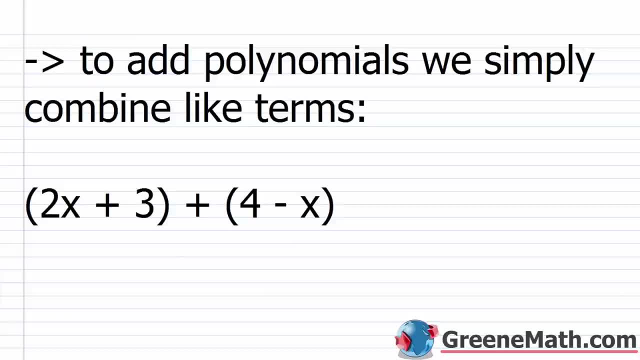 of this lesson. Once you get past all the kind of vocabulary stuff that you have to learn, it's really really easy to add and subtract polynomials. So to add polynomials, we simply combine like terms. We've been doing this since the beginning of algebra Super. 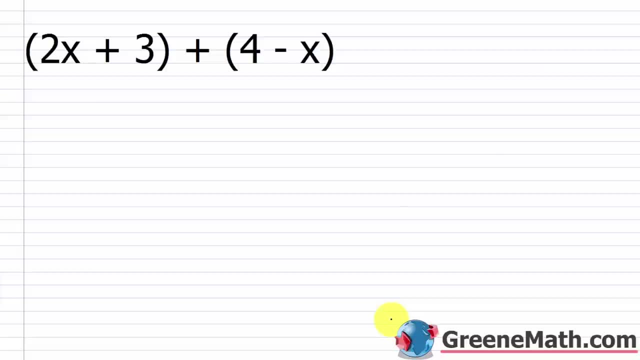 super simple at this point. So we have 2x plus 3- that polynomial- plus 4 minus x- that polynomial. So you can add this vertically if you want. A lot of students like to do that, They'll go. okay, I have 2x plus 3 and I have. you could rearrange this and say I have negative x plus 4 and you can kind of 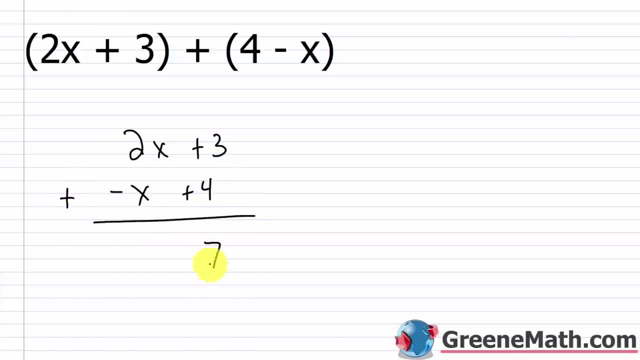 add like this, because you're adding like terms. So 3 plus 4 is 7.. 2x plus negative x or 2x minus x is x. So your result would be x plus 7 or kind of more traditionally, and what I just like to do. 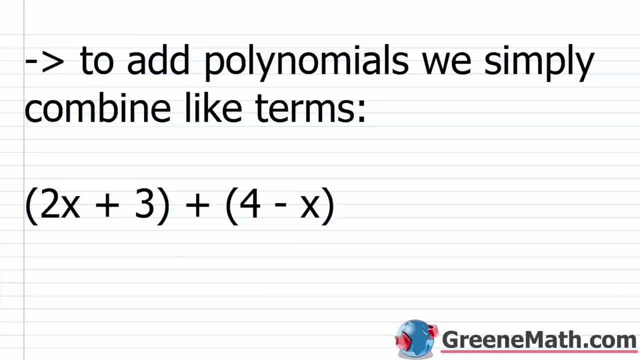 Alright, so now let's get to the meat of the lesson. And this is actually the easiest part of this lesson. 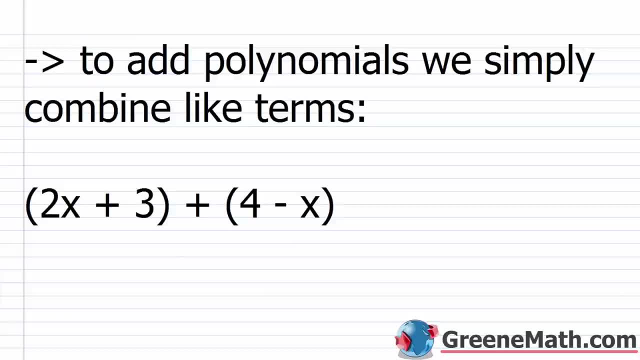 Once you get past all the kind of vocabulary stuff that you have to learn, it's really, really easy to add and subtract polynomials. So to add polynomials, you're going to have to do this. So to add polynomials, we simply combine like terms. We've been doing this since the beginning of algebra. Super, super simple at this point. 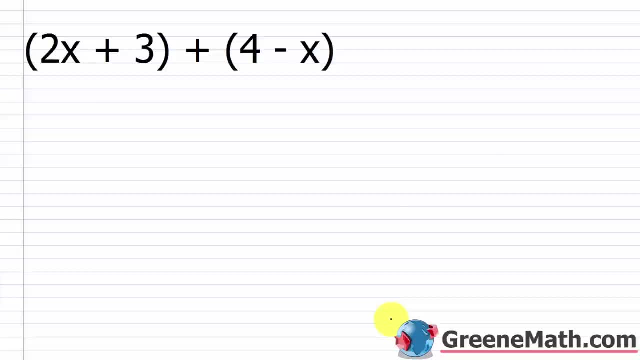 So we have 2x plus 3, that polynomial, plus 4 minus x, that polynomial. So you can add this vertically if you want. A lot of students like to do that. They'll go, okay, I have 2x plus 3, and I have... You could rearrange this and say I have negative x plus 4. And you can kind of add like this because you're adding like terms. So 3 plus 4 is 7. 2x plus 4 is 7. 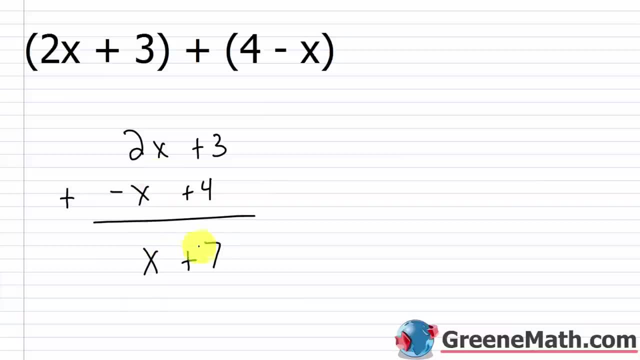 2x plus negative x or 2x minus x is x. So your result would be x plus 7. 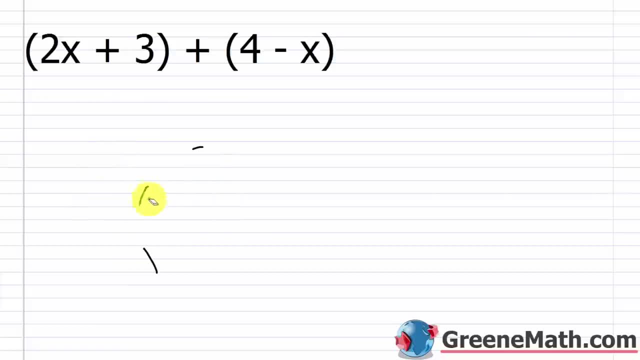 Or kind of more traditionally, and what I just like to do, you could just rearrange the terms. So I could just put like terms next to each other. So I'd have 2x plus negative x and then plus 3 plus 4. And then just combine like terms. 2x and negative x are like terms. Again, you keep the variable part the same. So the x stays the same. 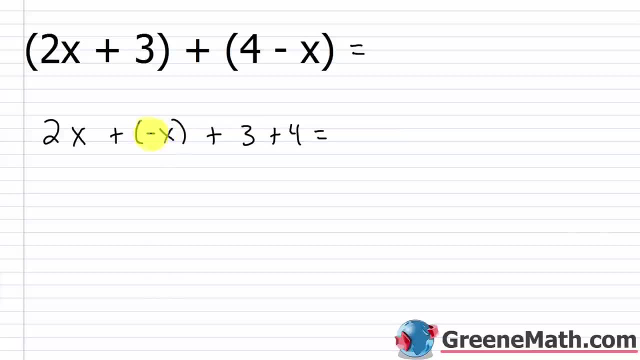 And I just add the coefficients. So here my coefficient, because I just have a negative there, is negative 1. So 2 plus negative 1 or 2 minus 1 is 1. So I would have 1x or just x from combining like terms here. So this would just be x. And then obviously 3 plus 4 is 7. So plus 7. Again, super, super easy. All right, so we have 5n squared minus n cubed. 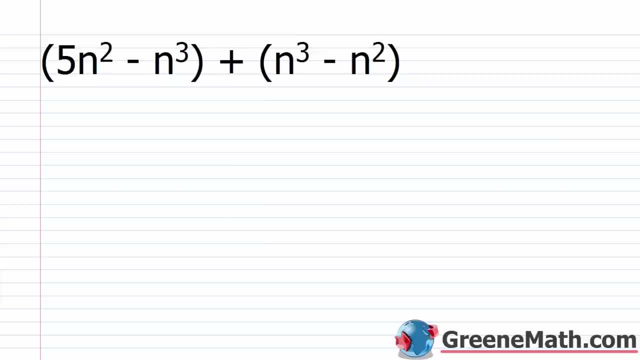 And we're adding to this n cubed minus n squared. So again, just put your like terms next to each other. So I have 5n squared and I have negative n squared. So I'd have 5n squared. You can put minus n squared or you can put plus negative n squared. It doesn't matter. And then I have minus n cubed and I have plus n cubed. So everything is written next to each other. So these are like terms, same variable, same power. 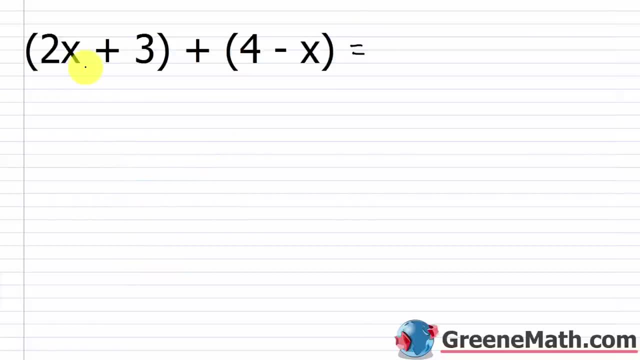 you could just rearrange the terms So I could just put like terms next to each other, So I'd have 2x plus negative x and then plus 3, plus 4 and then just combine like terms. 2x and negative x are like terms. Again, you keep the variable part. 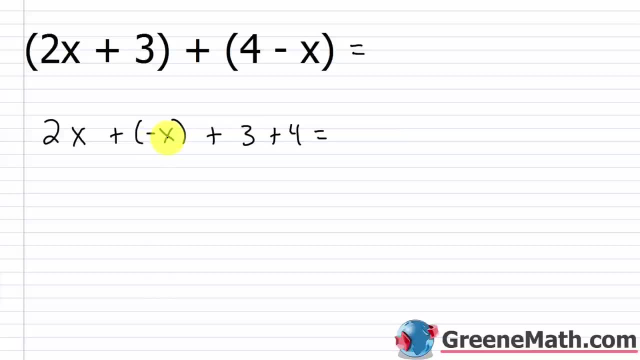 the same. So the x stays the same and I just add the coefficients. So here my coefficient: because I just have a negative, there is negative 1.. So 2 plus negative 1 or 2 minus 1 is 1.. So I would have. 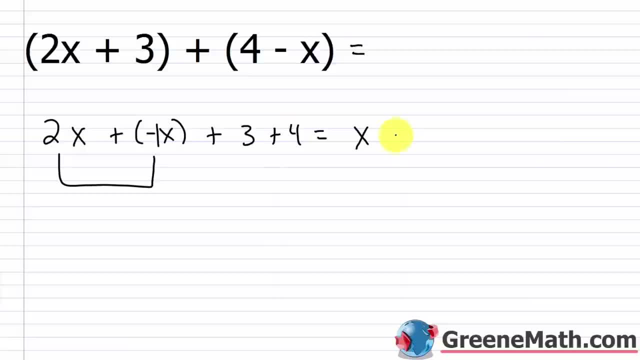 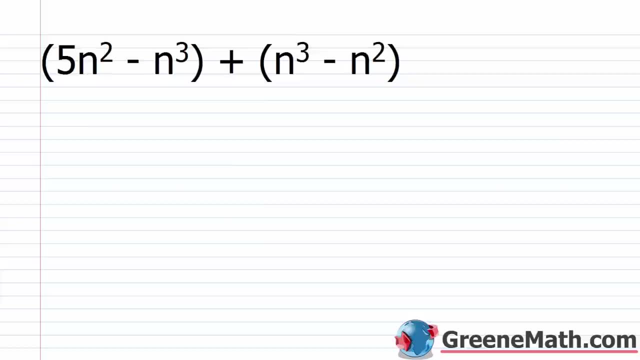 negative 1.. So this would just be x, and then obviously 3 plus 4 is 7.. So plus 7. Again, super, super easy, All right. so we have 5n squared minus n cubed, and we're adding to this n cubed minus n. 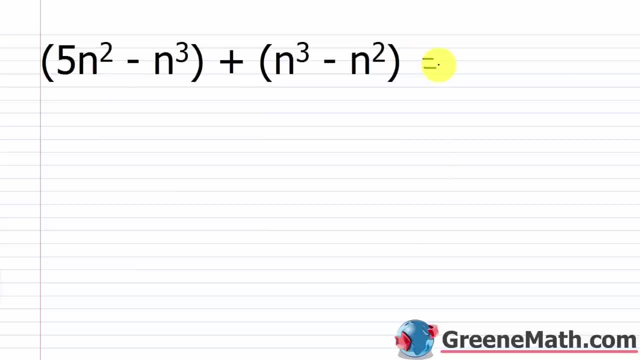 squared. So again, just put your like terms next to each other. So I have 5n squared and I have negative n squared. So I'd have 5n squared. You can put minus n squared, or you can put plus negative n squared, It doesn't matter. And then I have minus n cubed, minus n squared, So I'd have 5n squared. 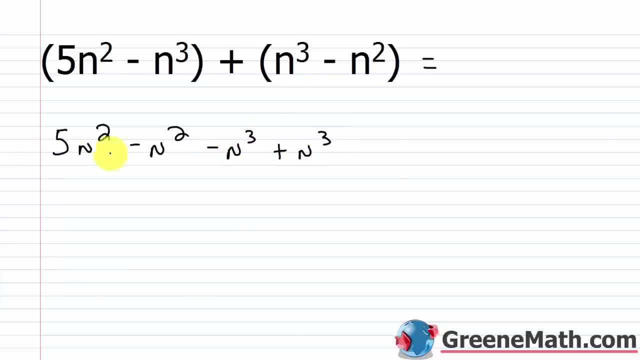 And I have plus n cubed, Okay, so everything's written next to each other. So these are like terms, Same variable, Same power. And then these are like terms, Same variable, Same power. So again I'm just going to say: 5n squared minus n squared is what, That's: 4n squared, The variable. 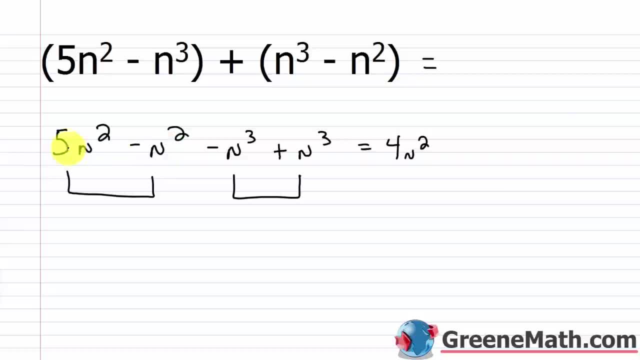 part n squared stays the same, and I'm just subtracting coefficients. So the coefficient here is a 5.. The coefficient here is basically a negative 1.. 5 minus 1 is 4.. So that's how I got that 4.. 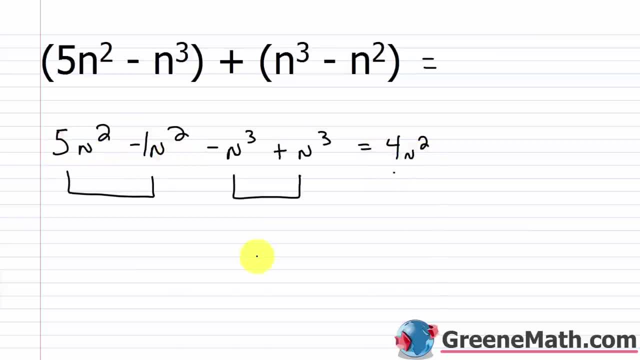 And then the variable part, n squared, stays the same. Then we have a negative n cubed plus a positive n cubed. This is basically like saying: I have negative 1 plus positive 1. That's 0.. Right, The variable part would stay the same, 0 times anything, though is 0. So it would basically cancel. 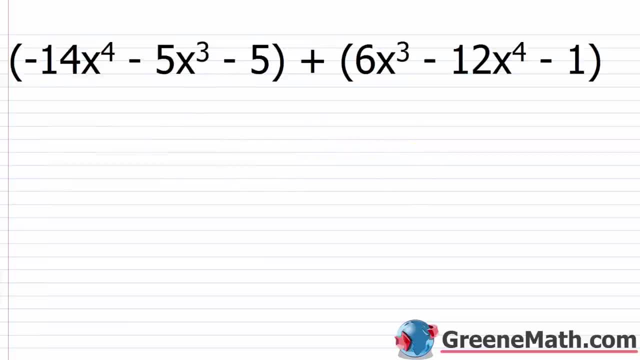 itself out, So we'll just have 4n squared as our answer. All right, now we're looking at negative 14x to the fourth power, minus 5x cubed, minus 5, plus 6x cubed, minus 12x to the fourth power. 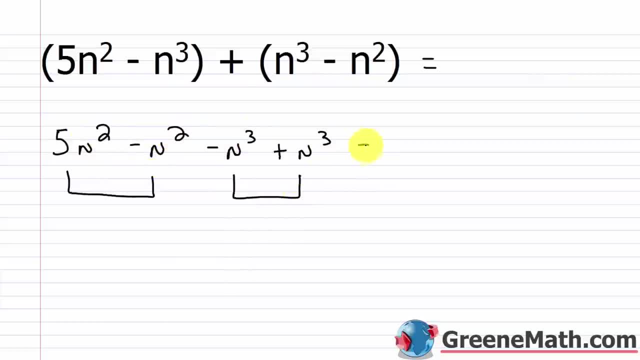 And then these are like terms, same variable, same power. So again, I'm just going to say 5n squared minus n squared is what? 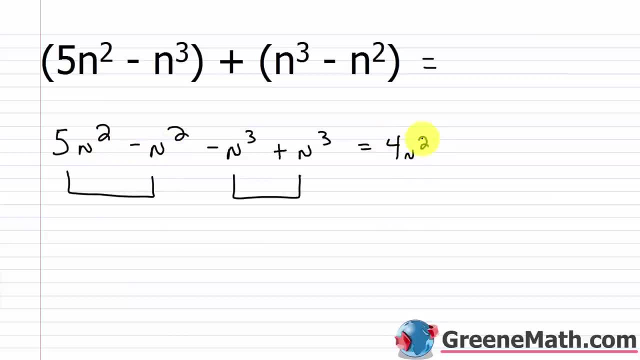 That's 4n squared. The variable part n squared stays the same. And I'm just subtracting coefficients. So the coefficient here is a 5. The coefficient here is basically a negative 1. 5 minus 1 is 4. So that's how I got that 4 there. 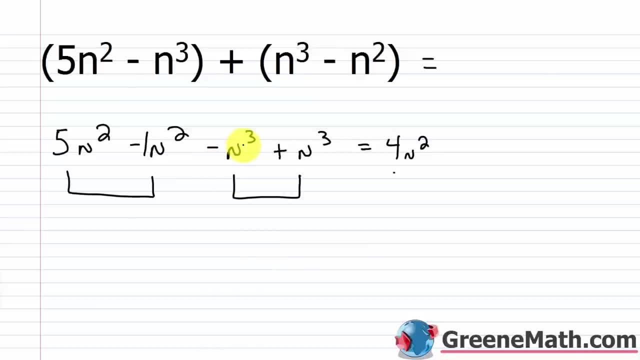 And then the variable part n squared stays the same. Then we have a negative n cubed plus a positive n cubed. This is basically like saying I have negative 1 plus positive 1. That's 0, right? The variable part would stay the same. 0 times anything, though, is 0. So it would basically cancel itself out. So we'll just have 4n squared as our answer. All right. 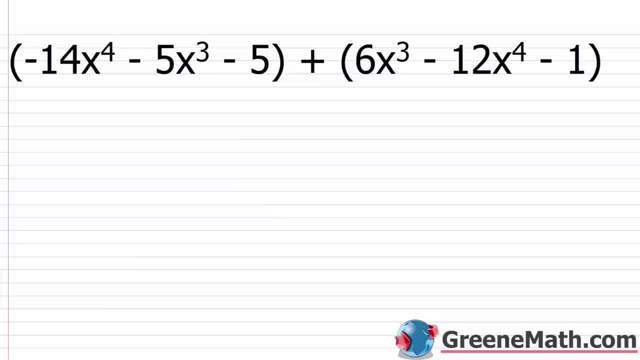 Now we're looking at negative 14x to the fourth power minus 5x cubed minus 5 plus 6x cubed minus 12x to the fourth power minus 1. So I'm just going to start out again by just writing my like terms next to each other. So I have negative 14x to the fourth power. I have minus 12x to the fourth power. I have negative 5x cubed. I have plus 6x cubed. Then I have minus 5 and then minus 1. So these are like terms, these are like terms, and these are like terms. So that's what I can combine. 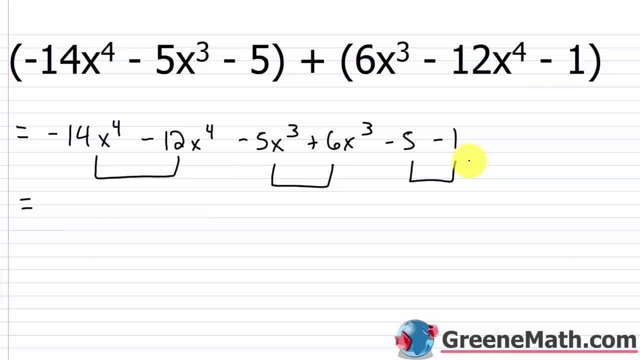 So negative 14x to the fourth power minus 12x to the fourth power. Again, x to the fourth power stays the same. I just add the coefficients. So negative 14 minus 12 is going to be negative 26. So this would be negative 26x to the fourth power. 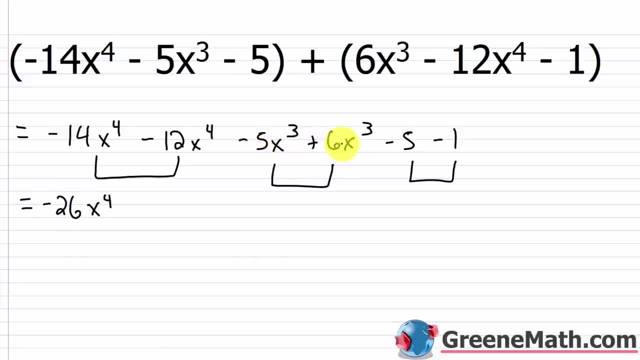 And then if I look at negative 5x cubed plus 6x cubed, x cubed is going to stay the same. I just add the coefficients. So what is negative 5 plus 6? That's 1. 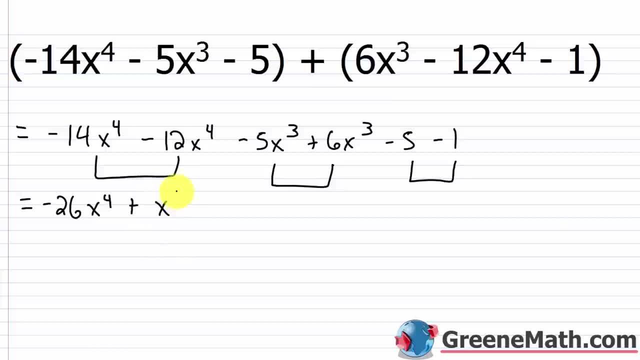 So this is going to be plus 1x cubed or just x cubed. And then lastly, I have negative 5 minus 1. And we know that's going to be negative 6. So then minus 6. 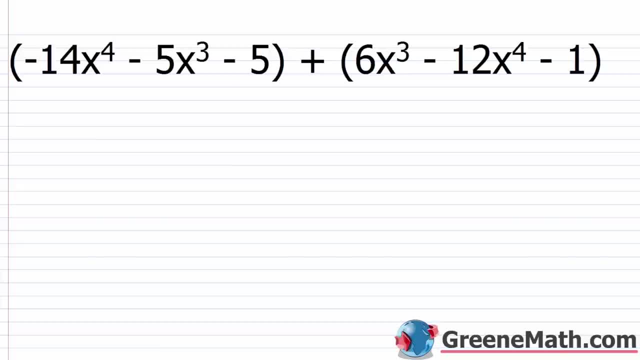 minus 1.. So I'm just going to start out again by just writing my like terms next to each other. So I have negative 14x to the fourth power, I have minus 12x to the fourth power, I have negative 5x cubed, I have plus 6x cubed, Then I have minus 5 and then minus 1.. So these are like terms, These. 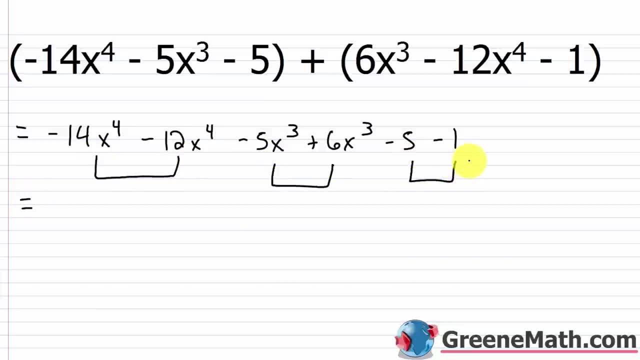 are like terms And these are like terms, So that's what I can combine. So negative 14x to the fourth power minus 12x to the fourth power, Again x to the fourth power stays the same. I just add the coefficients. So negative 14 minus 12 is going to be negative 26.. So this 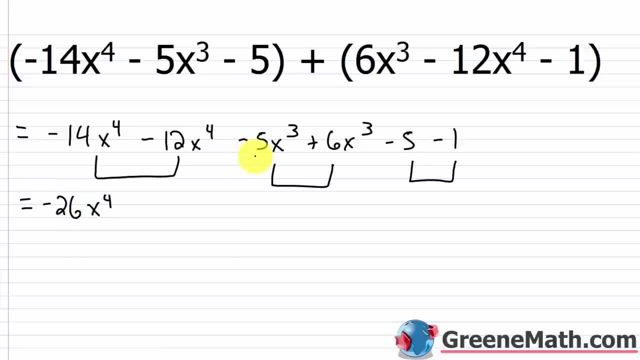 would be negative 26x to the fourth power. Then if I look at negative, 5x cubed plus 6x cubed, x cubed is going to stay the same, I just add the coefficients. So what is negative? 5 plus 6?? 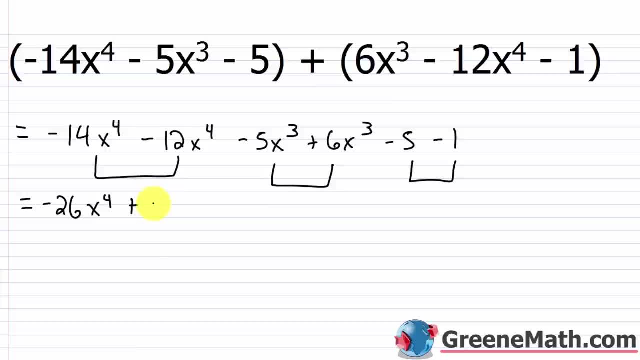 That's 1.. So this is going to be plus 1x cubed or just x cubed. And then, lastly, I have negative 5 minus 1. And we know that's going to be negative 6. So then, minus. 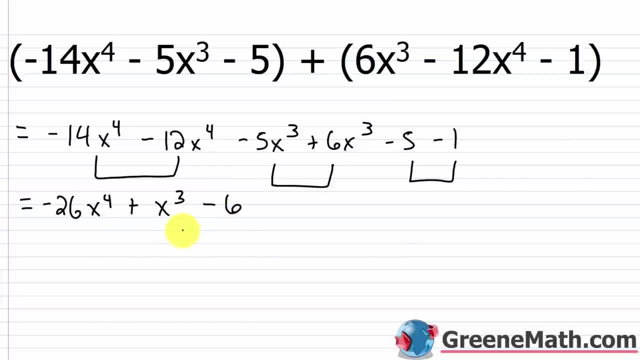 6. And this is already written in standard form, Kind of when I think about doing this process a lot of times, I'll just set it up to where my results are going to be, in descending order. Sometimes I forget and don't do that, But if you notice that it's out of order, you can quickly 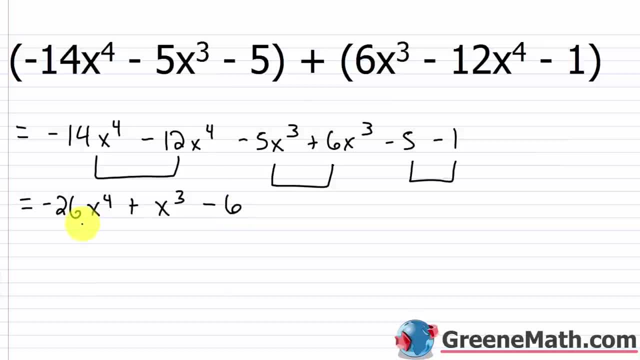 just rearrange it. It's easy to tell: okay, this term is of the highest degree. Then this is the sense of what is the x cubed and what is the 0. It's not if you do it the reverse way. So this: 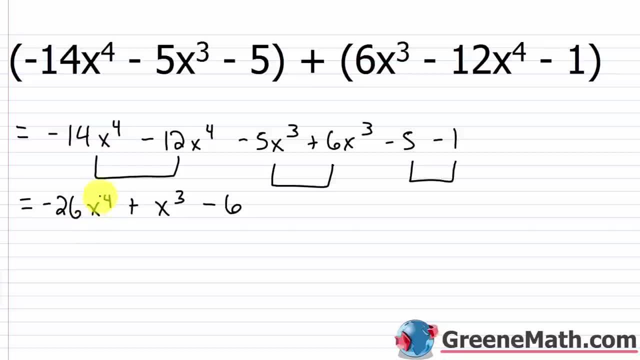 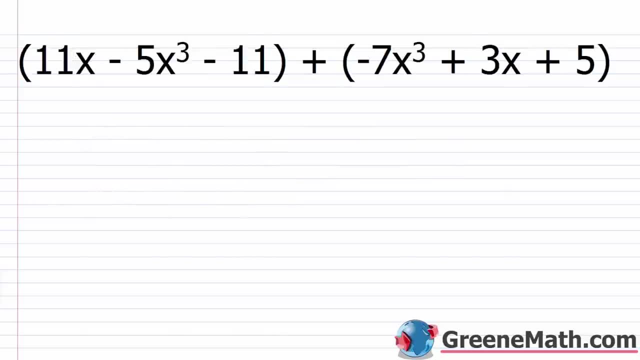 is what it's going to come down to. So I might not explicitly say it, but you know, for the terms of moving forward, you always want to try and write your polynomials in standard form, And that just means that, okay, I have x to the fourth power here, followed by x to the third power, followed. 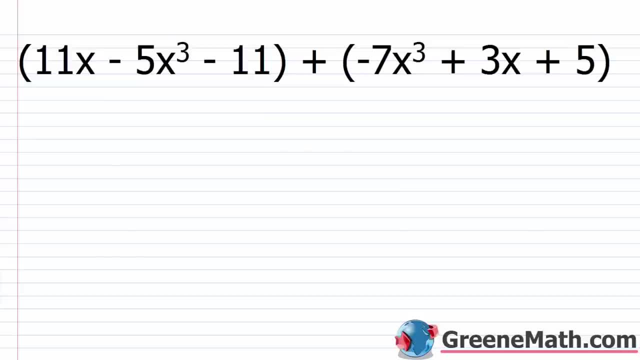 by x to the power of 0, right, so on and so forth. Alright, now I have 11x minus 5x cubed minus 11, plus I have negative 7x cubed plus 3x plus 5.. have 9.. 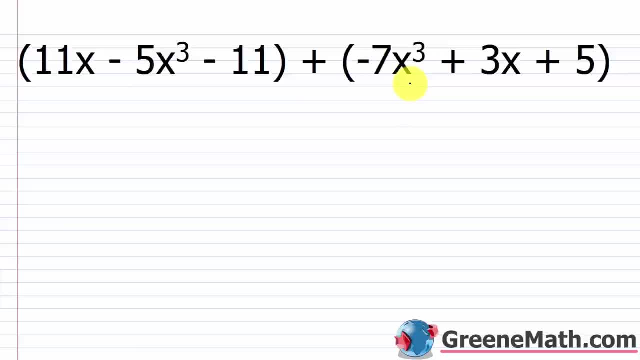 So I could start out with that one if I wanted to, or I could just rearrange it at the end, It doesn't really matter. So I can just say: okay, I have 11x and then plus 3x, and then I have negative 5x cubed. 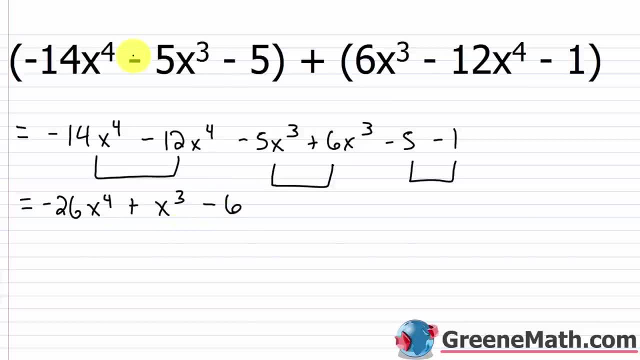 And this is already written in standard form. Kind of when I think about doing this process, a lot of times I'll just set it up to where my results are going to be in descending order. 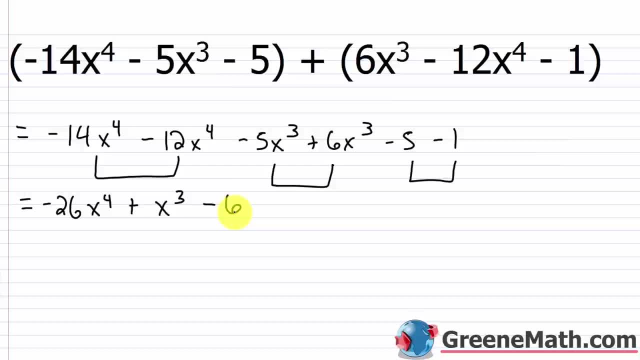 Sometimes I forget and don't do that. But if you notice that it's out of order, you can quickly just rearrange it, right? It's easy to tell, okay, this term is of the highest degree. 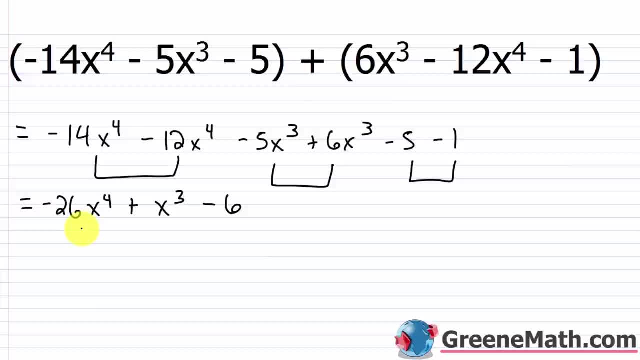 Then this is the second highest degree, you know, so on and so forth. So your teacher might not explicitly say it, but, you know, for the terms of moving forward, you always want to try and write your polynomials in standard form. And that just means that, okay, I have x to the fourth power here. Followed by x to the third power. Followed by, you know, x to the power of 0, right? So on and so forth. 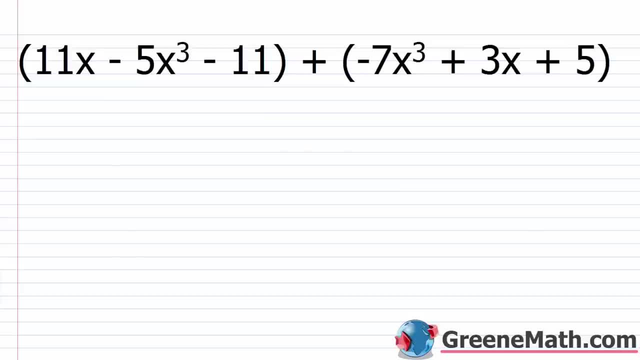 All right, now I have 11x minus 5x cubed minus 11. Plus I have negative 7x cubed plus 3x plus 5. 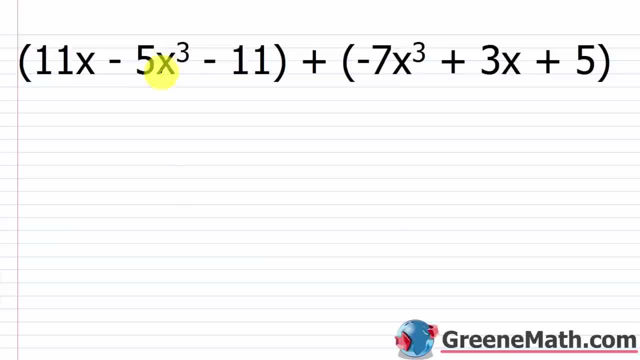 So if I wanted to, I know that this x cubed here is going to have the highest degree. So I could start out with that one if I wanted to. Or I could just rearrange it at the end. It doesn't really matter. 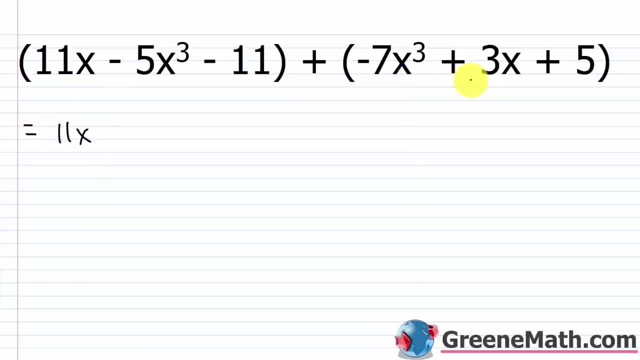 So I could just say, okay, I have 11x and then plus 3x. And then I have negative 5x cubed and then plus negative 7x cubed or minus 7x cubed. Then I have minus 11 and then plus 5. So I put the like terms next to each other. And because I wrote it this way, I'm going to have to rearrange my terms in the end so I put it in standard form. 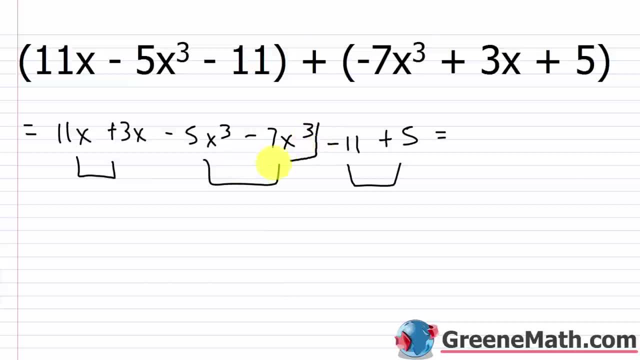 So if I wanted to save myself a little bit of work, I could have shifted this kind of down here, right? I could have started out with that. Okay, so moving forward. We have 11x plus 3x. 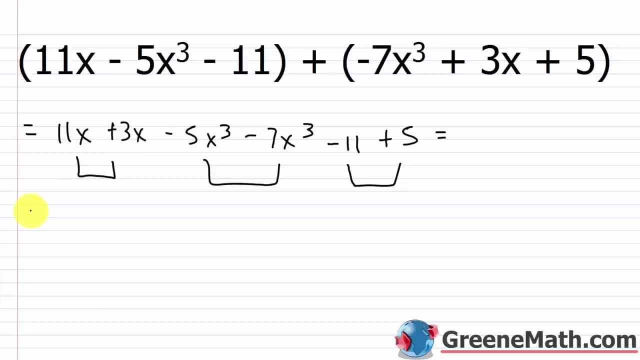 11 plus 3 is 14. x stays the same. So we get 14x. 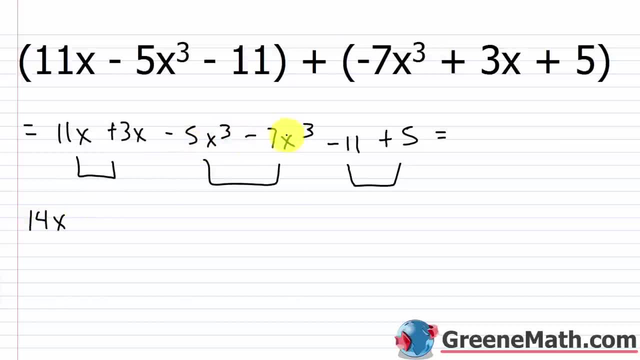 And then we have negative 5x cubed minus 7x cubed. Negative 5 minus 7 is negative 12. 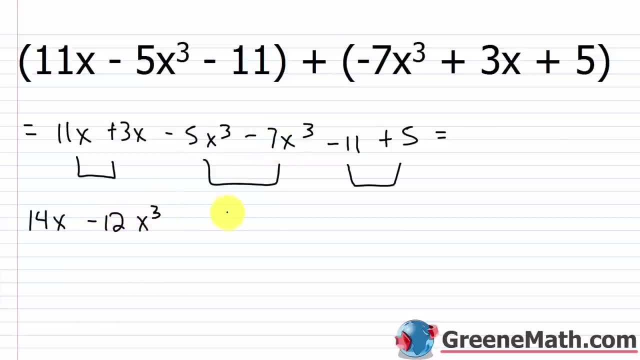 And then x cubed stays the same. And then we have negative 11 plus 5. That's going to be negative 6. So minus 6. 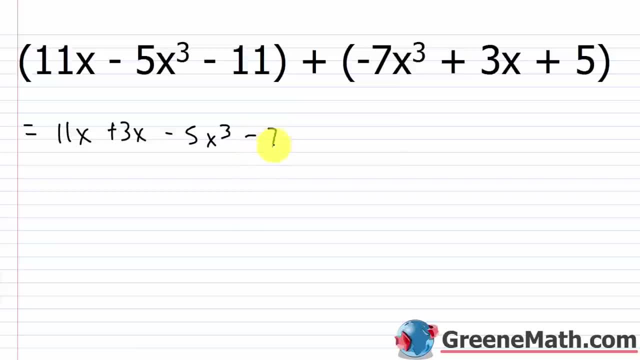 and then plus negative 7x cubed or minus 7x cubed, and I have minus 11, and then plus 5.. So I put the like terms next to each other And because I wrote it this way, I'm going to have to rearrange my terms in the end. 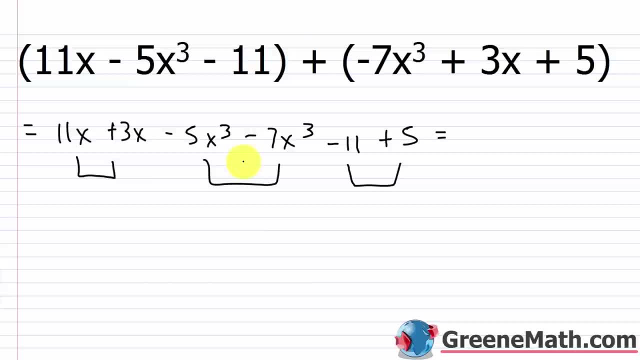 so I put it in standard form. So if I wanted to save myself a little bit of work, I could have shifted this kind of down here. right, I could have started out with that. Okay, so moving forward, We have 11x plus 3x. 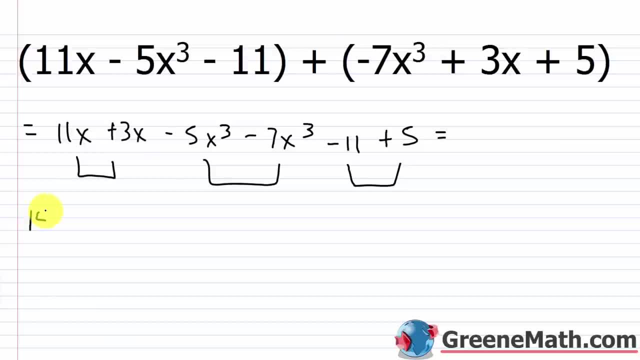 11 plus 3 is 14.. x stays the same, So we get 14x. and then we have negative 5x cubed minus 7x cubed. Negative 5 minus 7 is negative 12, and then x cubed stays the same. 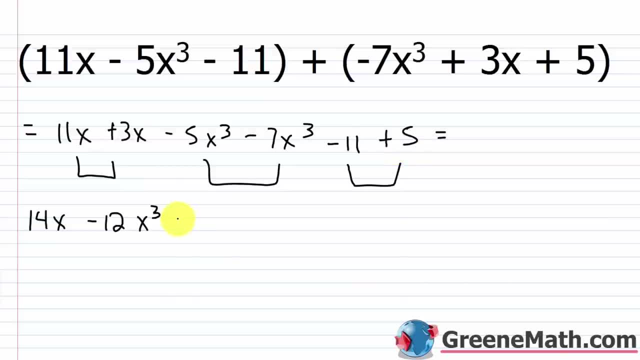 And then we have negative 11 plus 5. That's going to be negative 6.. So minus 6.. And this right now is again not in standard form, because this is x to the first power. This is x cubed. 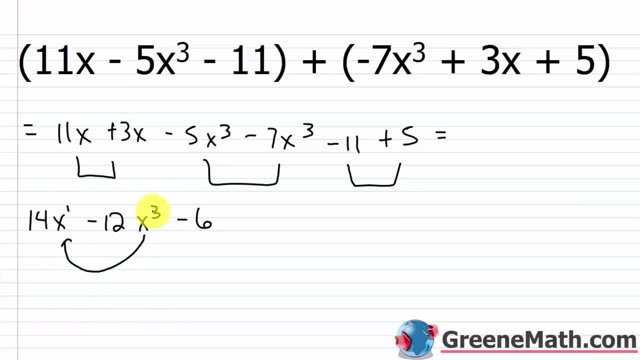 So this one has to go there. right. This has to go in the leading position because it's the term that has the highest degree. So we'd have negative 12x cubed out in front, and then plus 14x in second place, and then minus 6,. 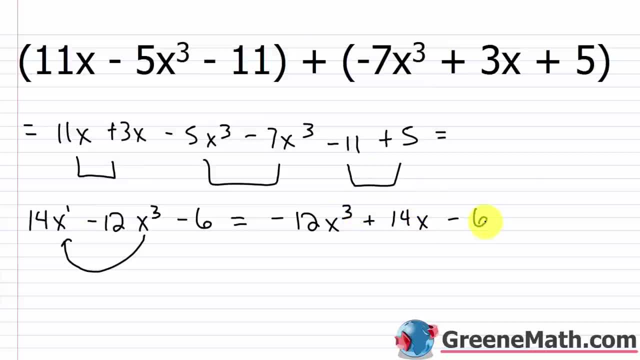 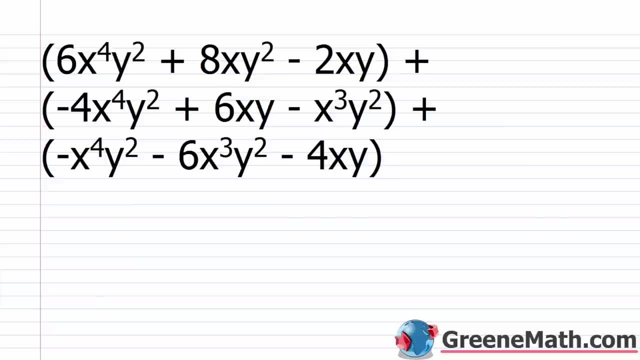 right: Highest degree, second highest degree, smallest degree. All right, let's look at one. It's a little bit harder and you might not see this in your textbook, but I wanted to throw this in there. You're going to get a lot of these in Algebra 2, where you have multiple, multiple variables. 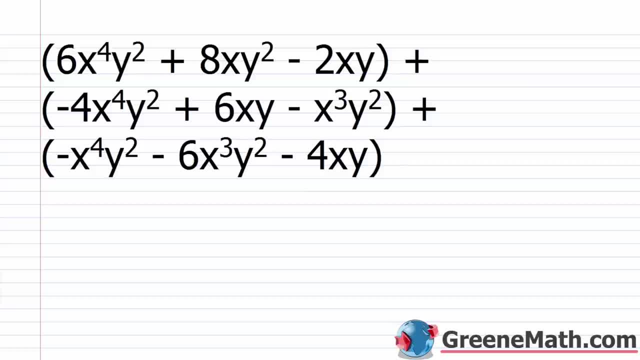 You might have five, six variables in there with all kinds of coefficients, And you know it's not any more difficult. It's just the fact that it's more tedious and you have to pay close attention to what you're doing. 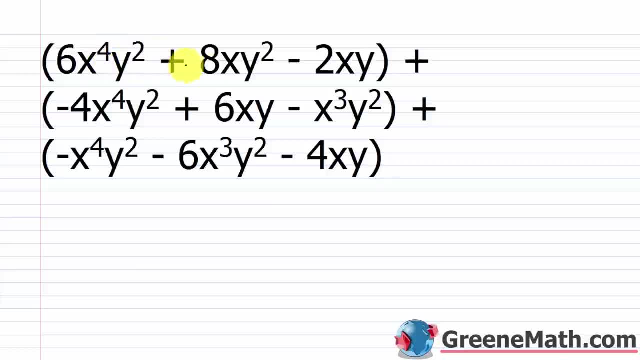 So we have 6x to the fourth power y squared plus 8xy squared, minus 2xy, plus negative 4x to the fourth power y squared plus 6x. So we're going to pay close attention to what the like terms are. so I'm going to start out with: we have 6x to the fourth power y squared, and every time I use something and put it over here, I'm going to go ahead and line it out, just so I know I've used it. 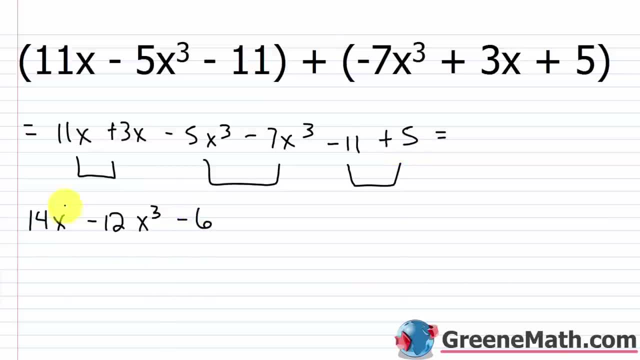 And this right now is, again, not in standard form because this is x to the first power. This is x cubed. So this one has to go there. Right? This has to go in the leading position because it's the term that has the highest degree. 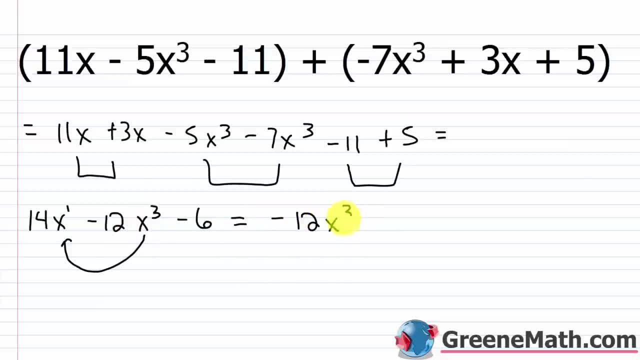 So we'd have negative 12x cubed out in front. And then plus 14x in second place. And then minus 6. Right? 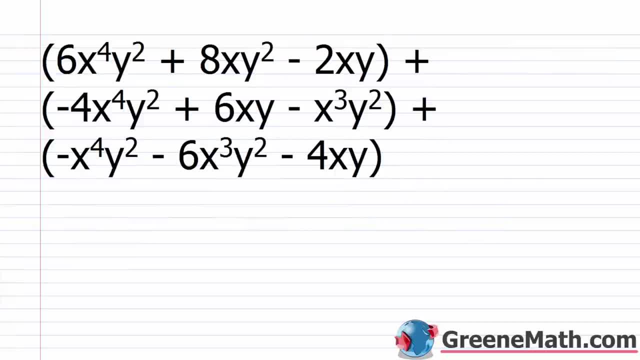 Highest degree. Second highest degree. Smallest degree. All right, let's look at one that's a little bit harder. And you might not see this in your textbook, but I wanted to throw this in there. 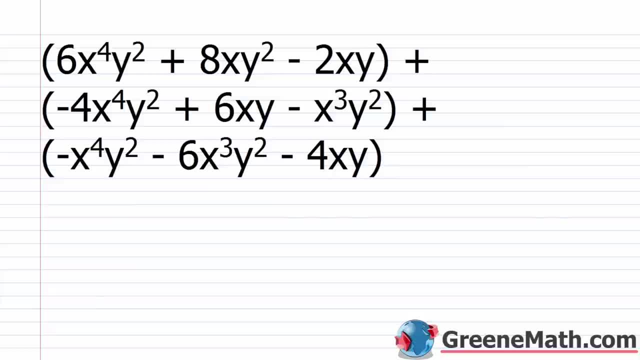 You're going to get a lot of these in Algebra 2 where you have multiple, multiple variables. You might have five, six variables in there with all kinds of coefficients. And, you know, it's not any more difficult. It's just the fact that it's more tedious. 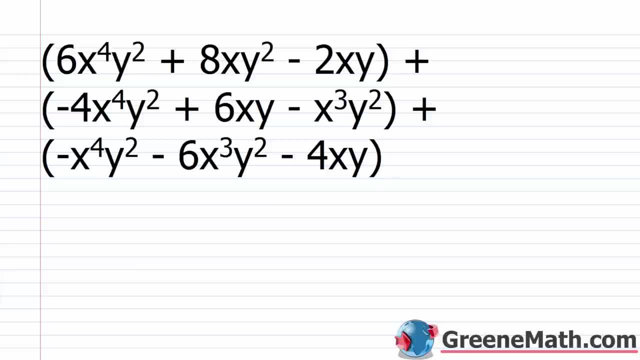 And you have to pay close attention to what you're doing. So we have 6x to the fourth power y squared plus 8xy squared minus 2xy plus negative 4x to the fourth power y squared plus 6xy minus x cubed y squared plus negative x to the fourth power y squared minus 6x cubed y squared. Minus 6x cubed y squared minus 4xy. 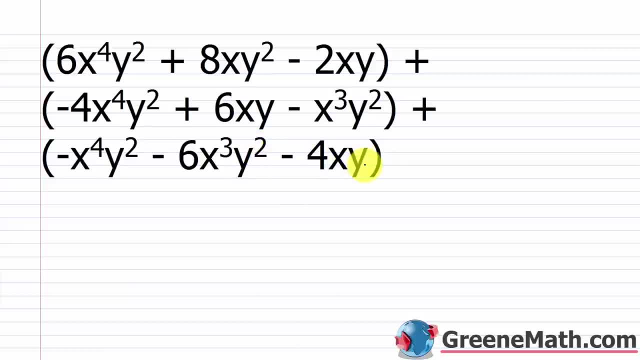 So we're going to pay close attention to what the like terms are. So I'm going to start out with we have 6x to the fourth power y squared. 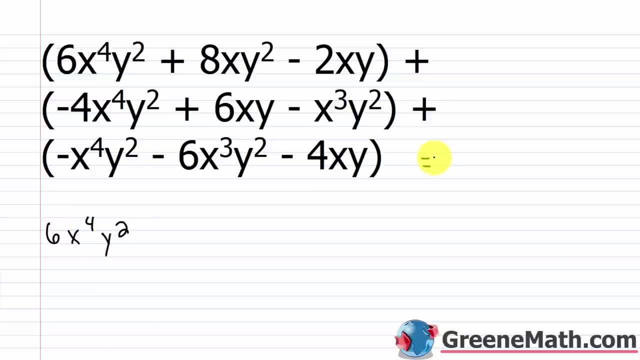 And every time I use something and put it over here, I'm going to go ahead and line it out. Just so I know I've used it, we can go back and erase that later just to keep track of what's going on. 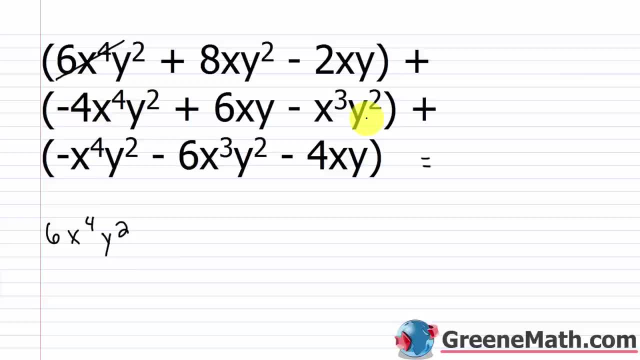 So then plus I have this term here in the other polynomial. So that's a negative 4x to the fourth power y squared. These are like terms. 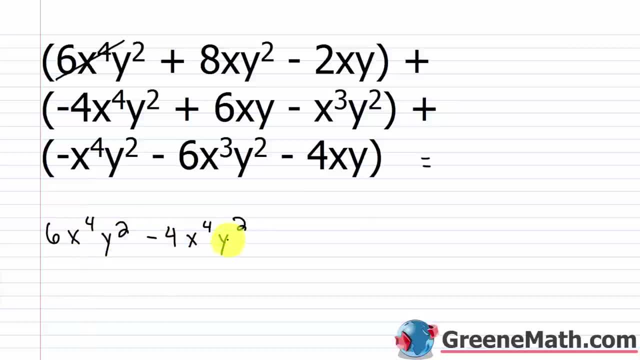 We have x to the fourth, x to the fourth. We have y squared and y squared. So those are going to be next to each other. 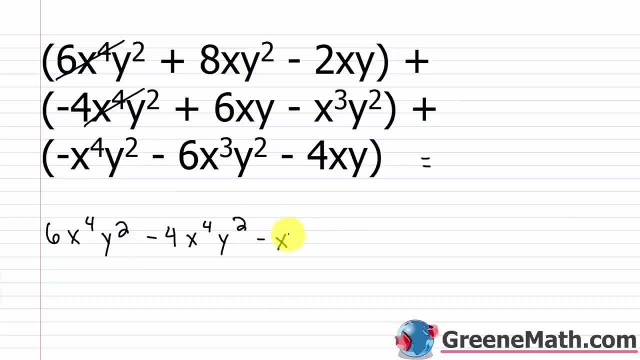 And then this one will be a like term also. We have minus x to the fourth power y squared. 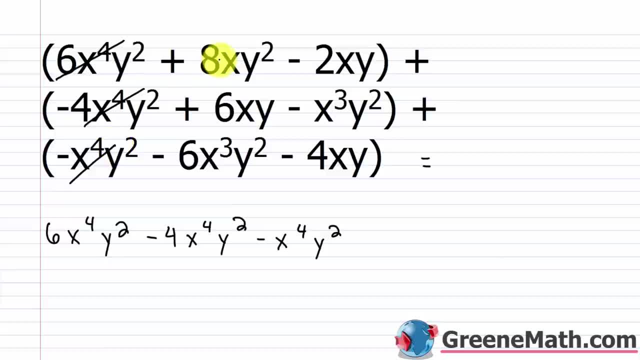 So I've used those three. Now, the next term in the first polynomial, I have 8xy squared. So 8xy squared. Any like terms with that. 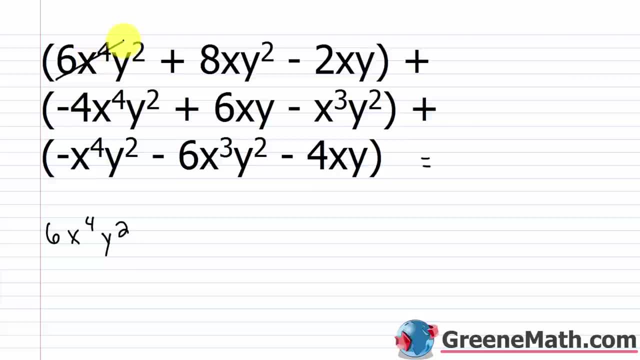 We can go back and erase that later, just to keep track of what's going on. So then, plus- I have this term here And the other polynomial, so that's a negative 4x to the fourth power, y squared. These are like terms. 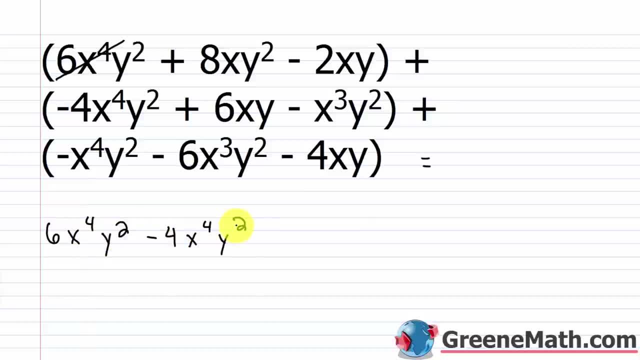 We have x to the fourth, x to the fourth, We have y squared and y squared, So those are going to be next to each other, And then this one will be a like term. also. We have minus x to the fourth power, y squared. 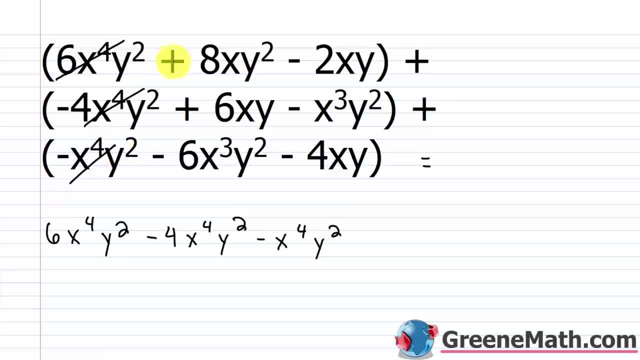 So I've used those three. Now the next term in the first polynomial I have 8xy squared, So 8xy squared Any like terms with that? I don't have an xy squared here. I don't have an xy squared here. 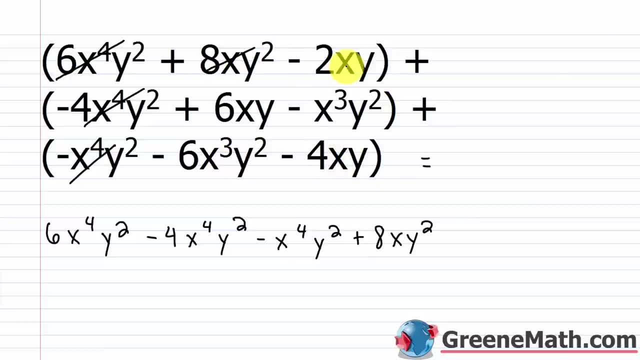 No xy squared anywhere else. So moving on Now. I have minus 2xy, So minus- let me kind of write this down here- Minus 2xy. So I've used everything from the first polynomial. In the second polynomial I have plus 6xy. 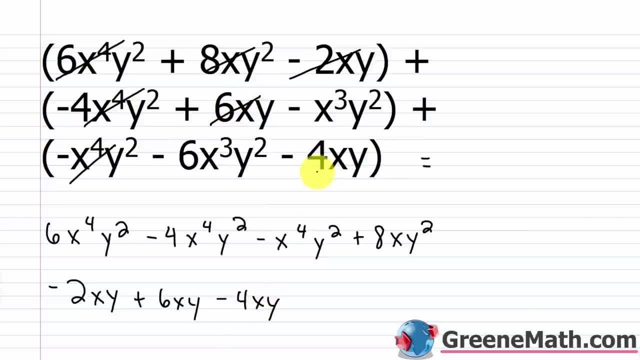 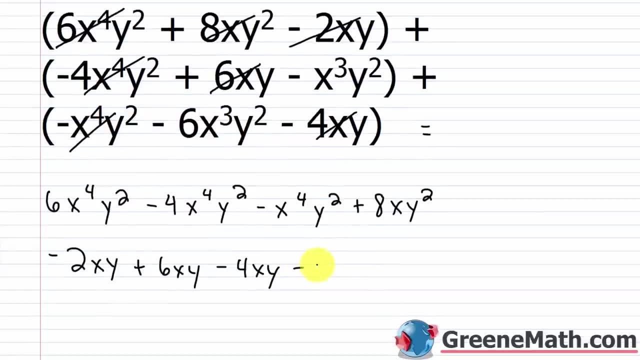 Line that out. In the third polynomial I have minus 4xy, So I've used all those. Okay, Now everything from the first polynomial is in here, The second polynomial: I still have a minus x cubed, y squared, And then I have that in the final polynomial as well. 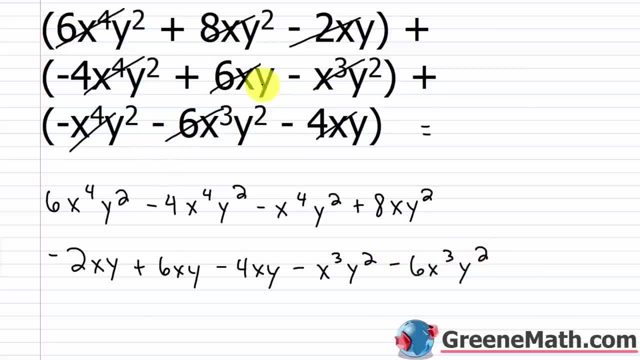 So minus 6x, cubed y squared, And so I've represented everything from all three polynomials in this, where all the like terms are next to each other, And once you've done that, you can go through and erase your little lines that you put in. 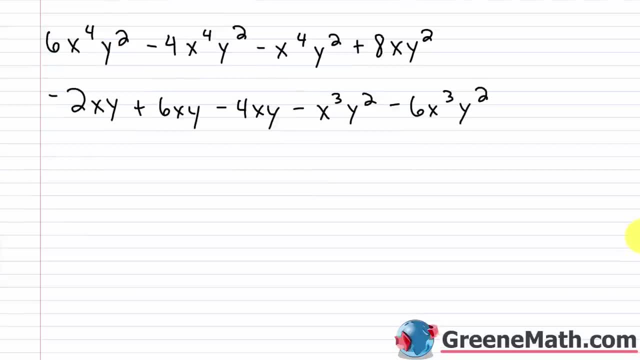 there. if you don't like to see that, Or you can leave it, It doesn't really matter. Okay, So now I'm going to combine like terms. So these three Are like terms, So just think about leaving the variable parts the same. 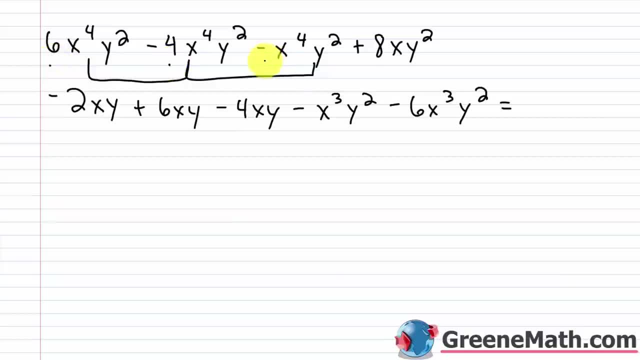 Just add the coefficients, So I have 6, negative 4, and negative 1. basically, So 6 plus negative 4 or 6 minus 4 is 2.. And then 2 minus 1 is 1.. So this would be 1 or just don't have to put anything. 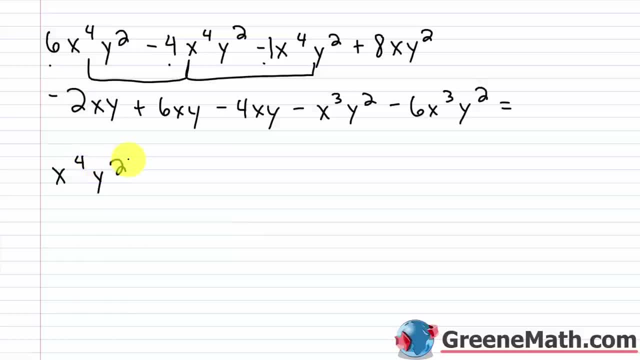 X to the fourth power, y squared. So I've taken care of these. And then next I have this: 8xy squared Plus 8xy. Okay, Plus 8xy squared. Nothing to match with that, Right? No like terms for that. 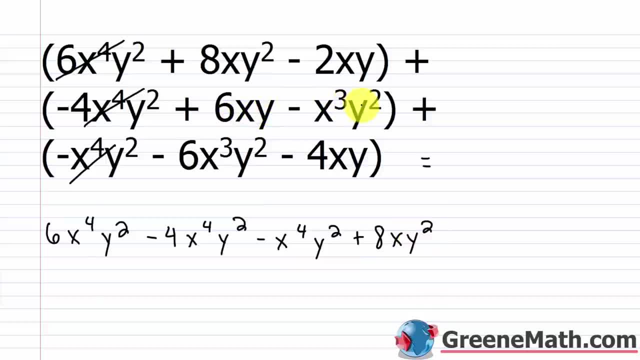 I don't have an xy squared here. I don't have an xy squared here. No xy squared anywhere else. So moving on. 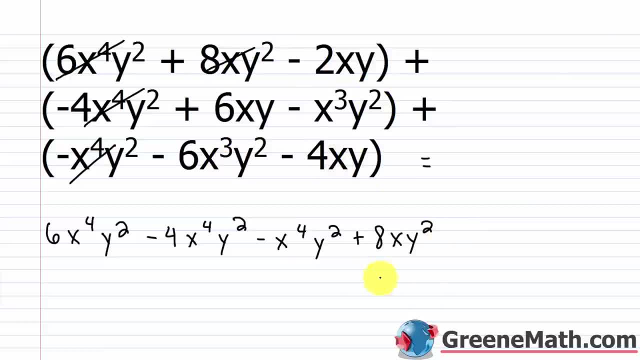 Now I have minus 2xy. So minus, let me kind of write this down here. Minus 2xy. So I've used everything from the first polynomial. 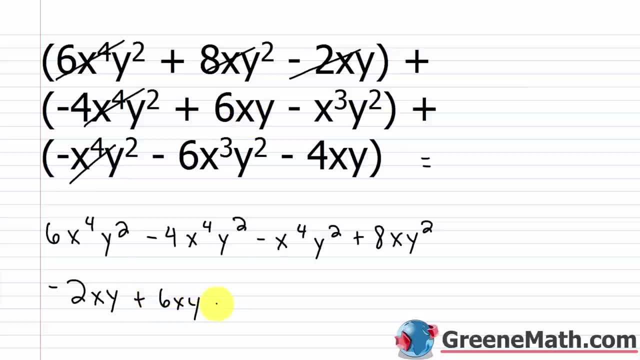 In the second polynomial, I have plus 6xy. Line that out. 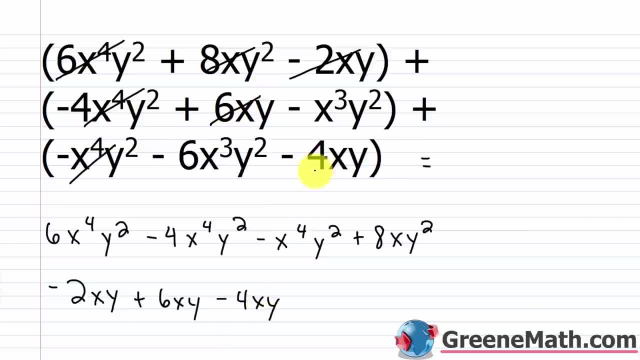 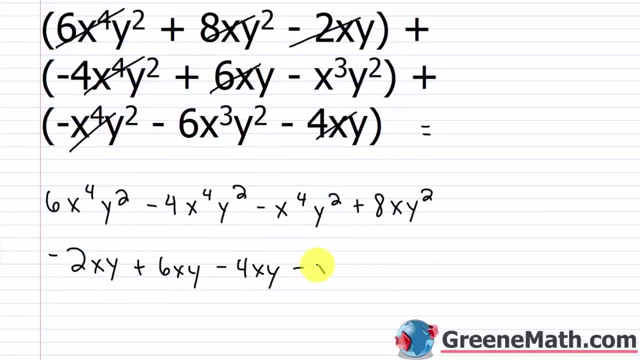 In the third polynomial, I have minus 4xy. So I've used all those. Okay. Now everything from the first polynomial is in here. The second polynomial, I still have a minus x cubed y squared. And then I have that in the final polynomial as well. So minus 6x cubed y squared. And so I've represented everything from all three polynomials in this where all the like terms are next to each other. 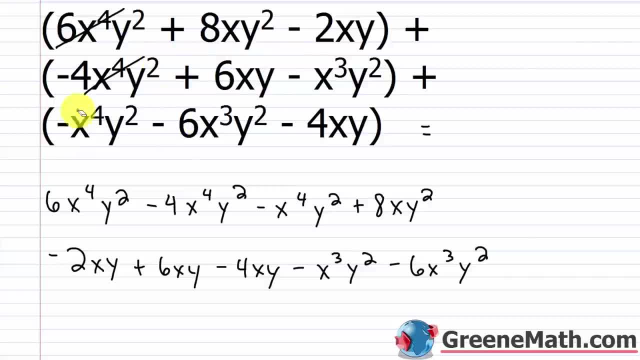 And once you've done that, you can go through and erase your little, you know, lines that you put in there if you don't like to see that. Or you can leave it. It doesn't really matter. Okay. So now I'm going to combine like terms. 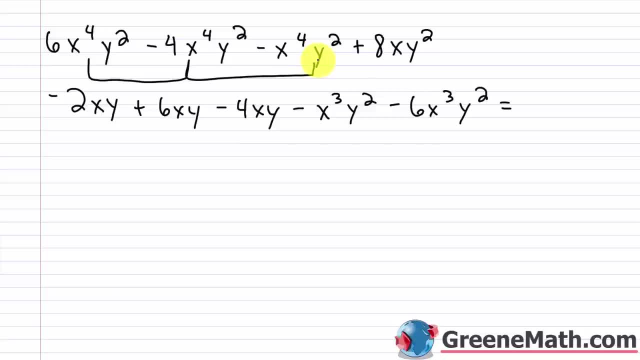 So these three are like terms. So just think about leaving the variable parts the same. Okay. Just add the coefficients. 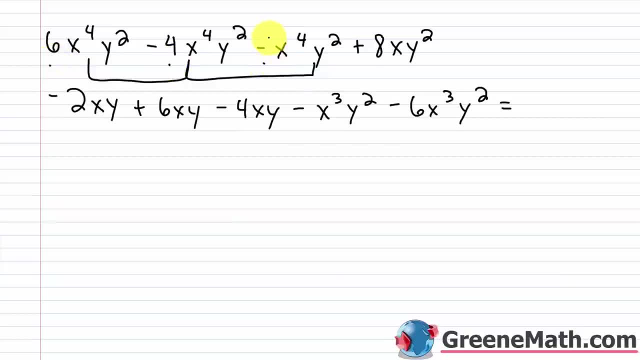 So I have 6, negative 4, and negative 1 basically. So 6 plus negative 4 or 6 minus 4 is 2. And then 2 minus 1 is 1. 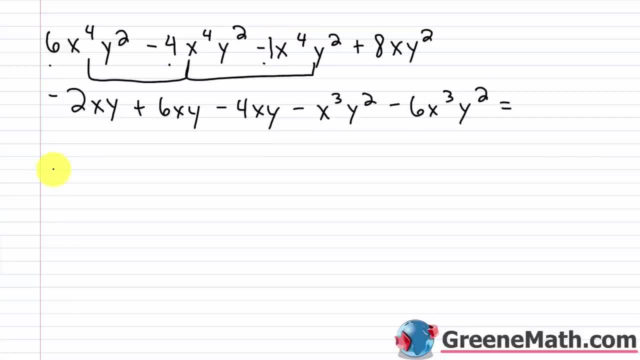 So this would be 1 or just don't have to put anything, x to the fourth power y squared. So I've taken care of these. 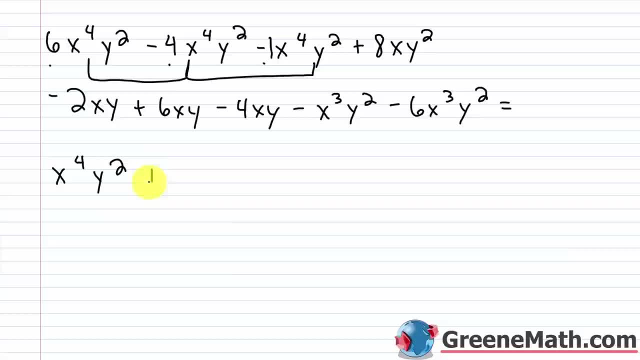 And then next I have this 8xy squared plus 8xy squared. Nothing to match with that, right? No like terms for that. And then here I have negative 2xy. 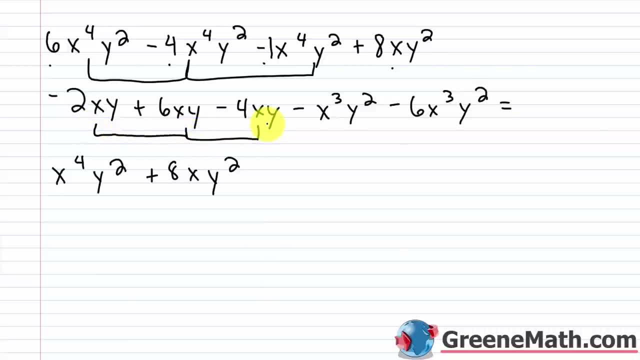 I have positive 6xy. And I have negative 4xy. So negative 2 plus 6 is 4. 4 minus 4 is 0. So what happened there? Those are going to be eliminated. Right? They're going to cancel each other out because 0 times anything is just 0. So these, you could line them out. Right? They cancel. 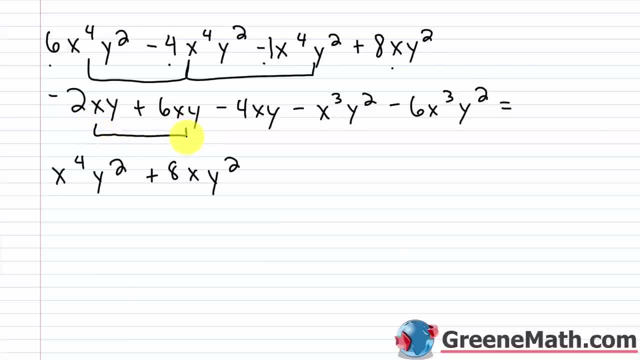 And then here I have negative 2xy, I have positive 6xy And I have negative 4xy, So negative: 2 plus 6 is 4.. 4 minus 4 is 0. So what happened there? Those are going to be eliminated. 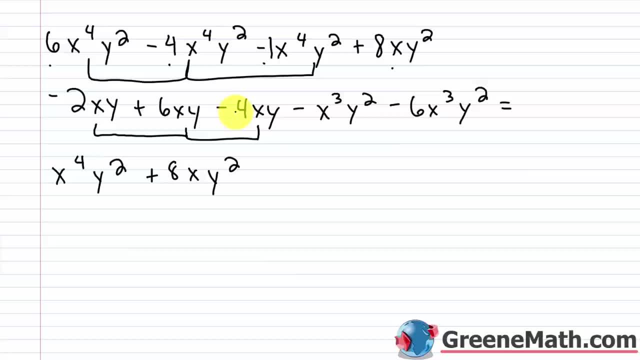 Right, They're going to cancel each other out, Because 0 times anything is just 0.. So these you could line them out: Right, They cancel. Then I'd have negative x cubed y squared Right, Minus 6x cubed y squared. 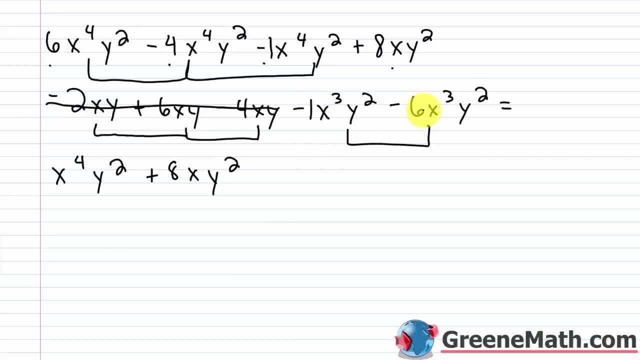 These are like terms, So I have basically negative 1 minus 6, which is negative 7.. So minus 7 times x cubed, y squared, And so this is our answer, But is it in standard form? Let's take a look. 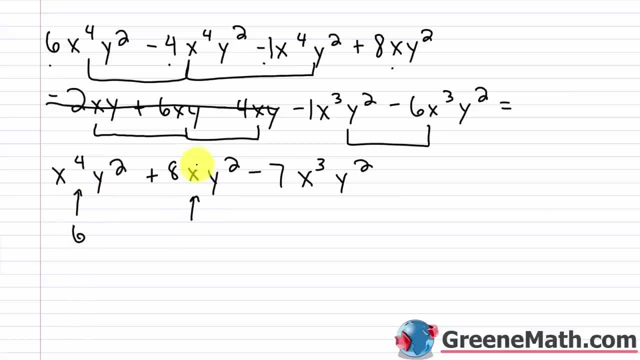 The degree for this term is 6.. The degree for this term- remember you have a 1 here- is 3.. And the degree for this term is 5.. So these are not in descending order, Right? So we're going to have to get switched with this. 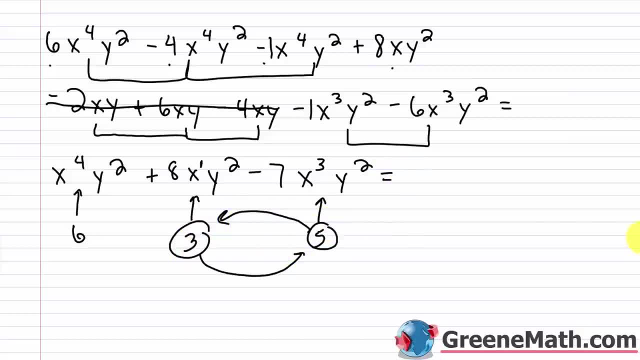 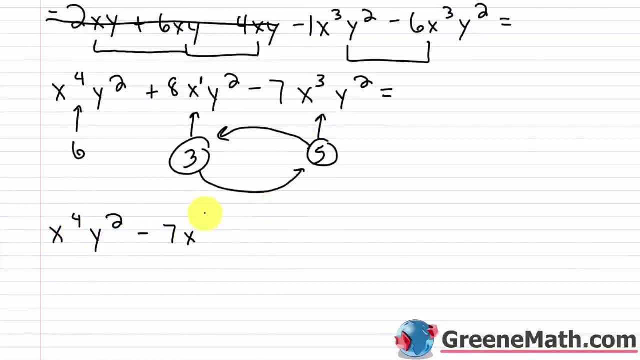 This needs to go here. So to write this in standard form, I would have x to the 4th power y squared, Then I would have minus 7x cubed y squared, And then I would have plus 8xy squared. 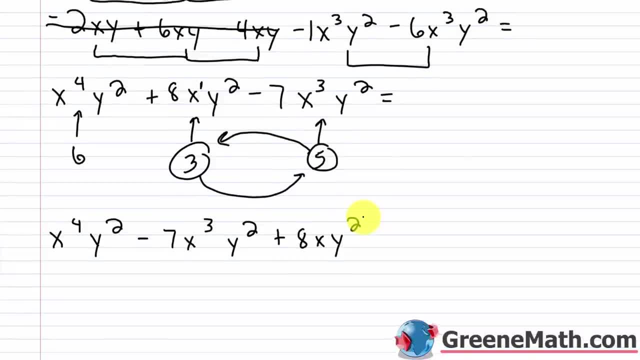 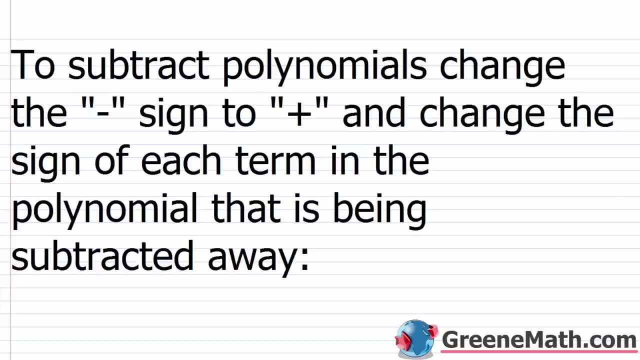 And once you get a little bit of practice with this, it becomes very, very easy. All right, So the next thing we're going to talk about is subtracting polynomials. So this is just as easy. There's just one additional step. 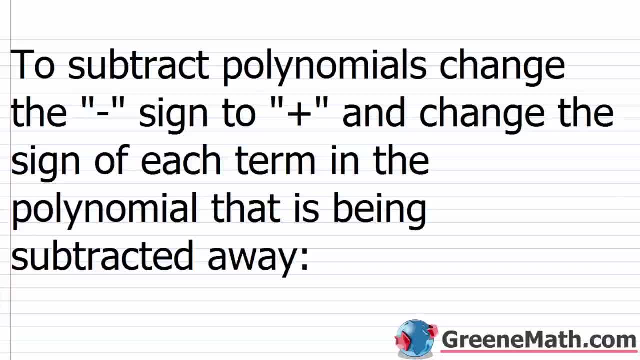 So to subtract polynomials, Change the minus sign to a plus sign And change the sign of each term in the polynomial that is being subtracted away. Very, very simple And goes back to this fundamental rule: If I have 2 minus 3.. 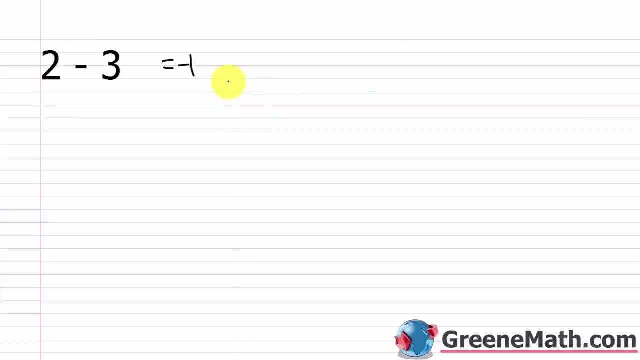 We know that's negative 1. This is the same thing as if I said it is 2 plus. Change this to plus And then change this to its opposite. It's the same thing as 2 plus negative 3. It's still negative 1.. 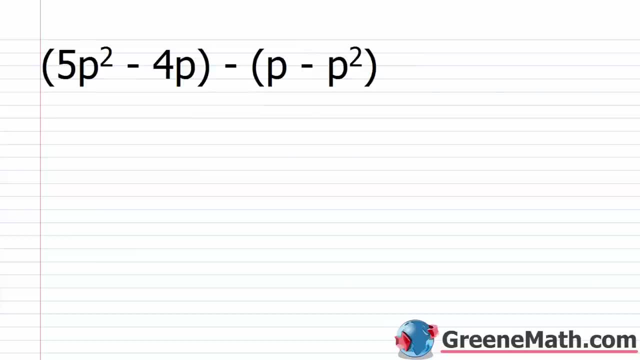 So that's all we're going to be doing here, using that same rule. So if I have 5p squared minus 4p, minus p, minus p, squared Again- you know this from earlier- If I see a minus sign out in front of a set of parentheses, in order to remove the parentheses, 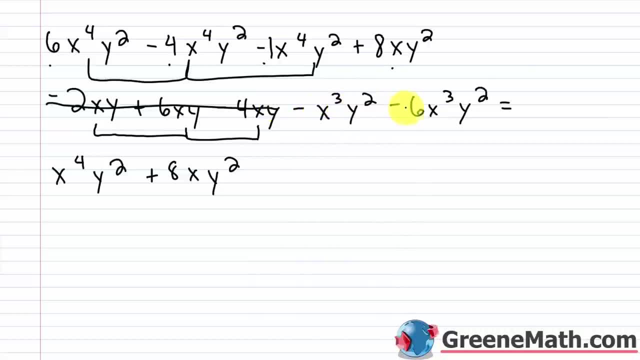 Then I'd have negative x cubed y squared minus 6x cubed y squared. These are like terms. So I have basically negative 1 minus 6, which is negative 7. 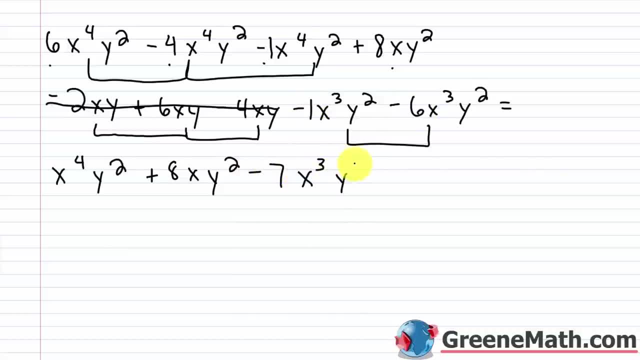 So minus 7 times x cubed y squared. 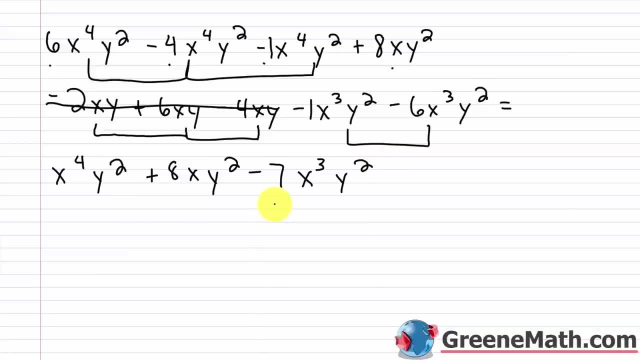 And so this is our answer, but is it in standard form? Let's take a look. The degree for this term is 6. 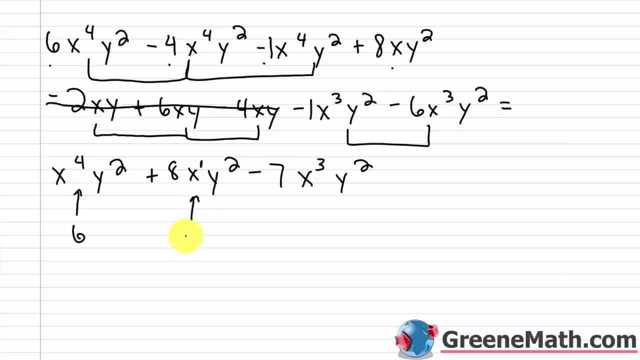 The degree for this term, remember you have a 1 here, is 3. And the degree for this term is 5. So these are not in descending order. Right? This needs to get switched with this. Right? 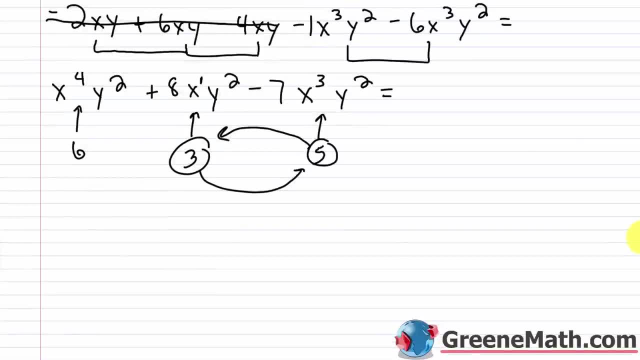 Let's take a look here. So to write this in standard form, I would have x to the fourth power y squared. Then I would have minus 7x cubed y squared. 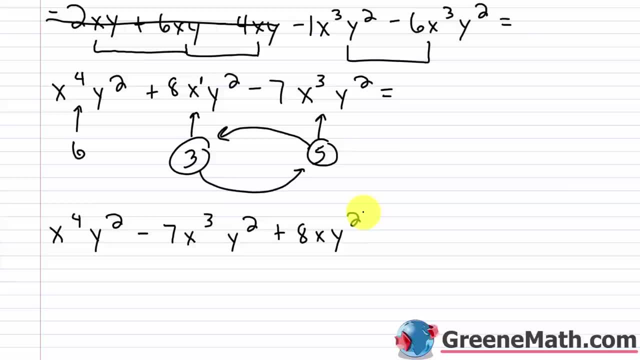 And then I would have plus 8xy squared. And once you get a little bit of practice with this, it becomes very, very easy. All right. 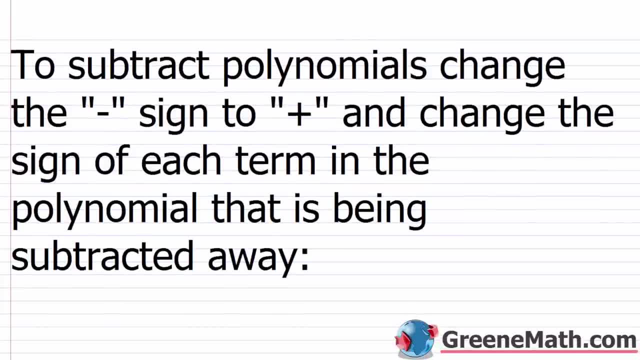 So the next thing we're going to talk about is subtracting polynomials. So this is just as easy. There's just one additional step. So to subtract polynomials, change the minus sign to a plus sign and change the sign of each term in the polynomial that is being subtracted away. 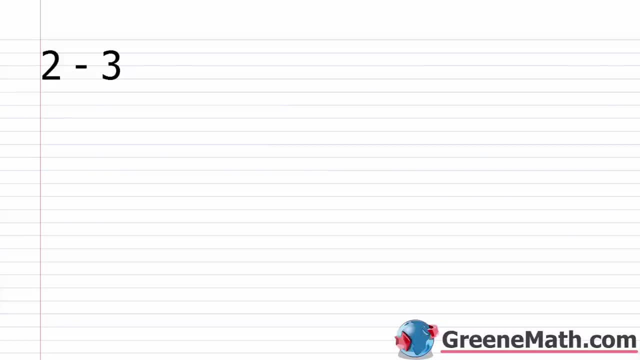 Very, very simple and goes back to this fundamental rule. If I have 2 minus 3, right, we know that's negative 1. This is the same thing as if I said it is 2 plus, right, change this to plus and then change this to its opposite. It's the same thing as 2 plus negative 3. It's still negative 1. So that's all we're going to be doing here using that same rule. 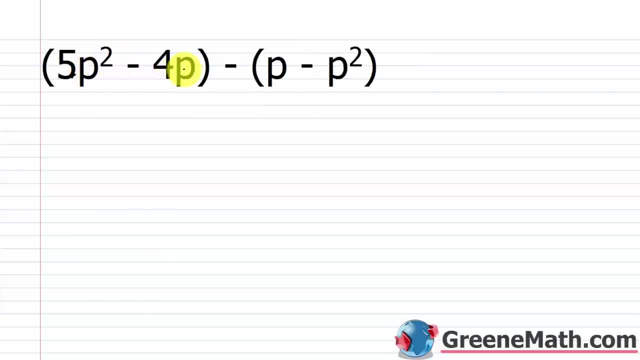 So if I have 5p squared minus 4p minus p minus p squared. Again, you know this from earlier. 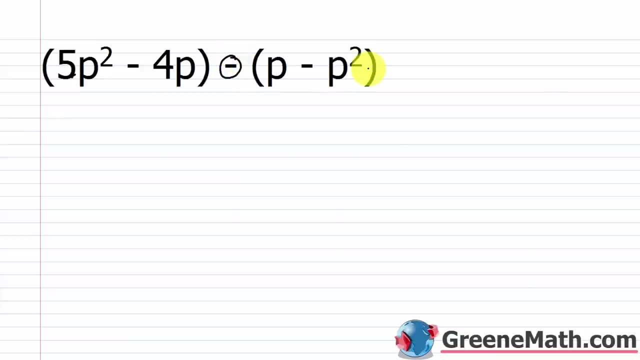 If I see a minus sign out in front of a set of parentheses, in order to remove the parentheses, again, you think about this as just multiplying by like a phantom negative 1. A lot of your teachers are going to say that. You change the sign of each term. So instead of p, that's going to be negative p. This is going to be negative p. 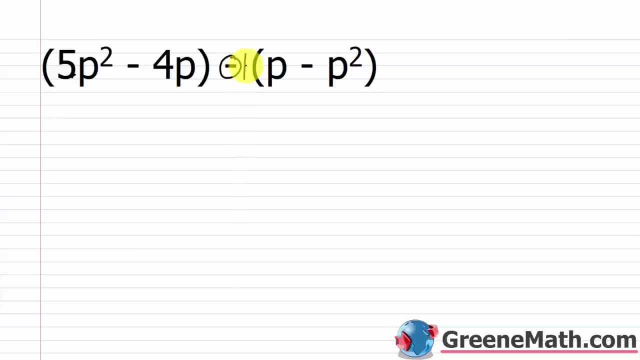 Again, you think about this as just multiplying by, like a phantom, negative 1. A lot of your teachers are going to say that you change the sign of each term. So instead of p- that's going to be negative p- This is going to be negative p. 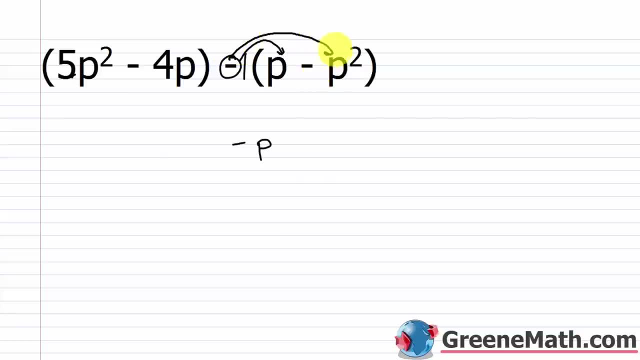 instead of negative p squared, you're going to change the sign. it's going to be plus p squared. so I would have 5p squared minus 4p and then minus p, plus p squared. okay, so if you're removing parentheses, you change the sign of each term inside the parentheses. that's just the rule. 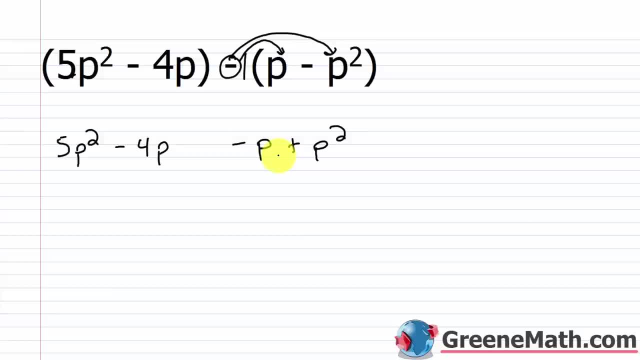 whether you're working with polynomials or or anything really. so now I can just set this up just like we did in the previous problems. so I have 5p squared plus p squared, put my like terms next to each other: minus 4p, minus p. so these are like terms and these are like terms. so 5p squared. 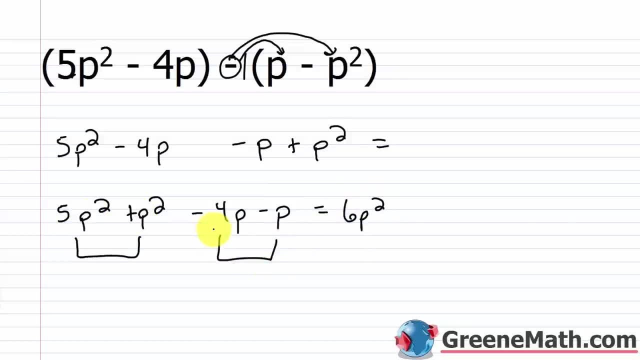 plus p squared, that's going to be 6p squared. and then negative 4p minus p, that's minus 5p. there's your answer: 6p squared minus 5p. again, whenever we see a negative outside of parentheses, a lot of teachers are just going to say, oh my god, I don't know how to do this. 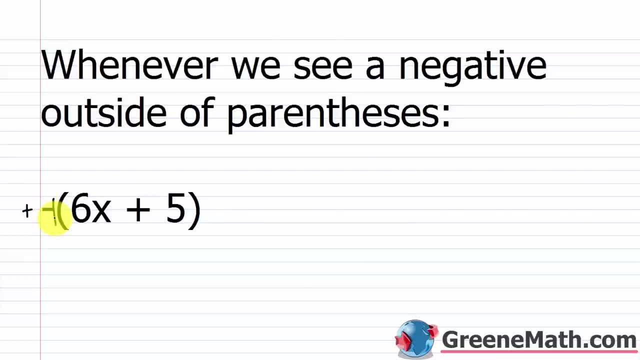 I'm just going to say: make this a plus negative 1 and distribute the negative 1. that's going to remind you to change the sign of everything. so this becomes negative 1 times 6x or negative 6x. negative 1 times 5 or minus 5. so that's just a rule to remember, just moving forward again, not 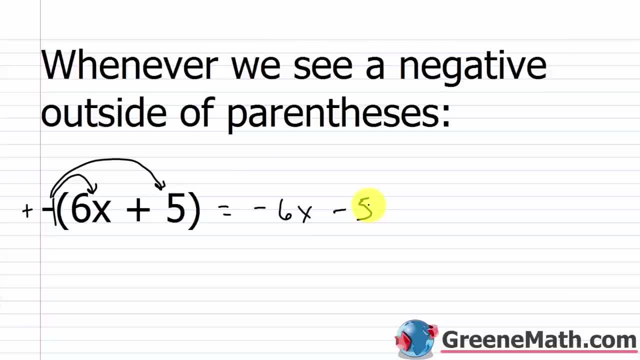 just when you're working with polynomials, but when you're just working in math in general. negative outside of parentheses. change the sign of each term inside the parentheses to drop the parentheses, all right. so now I'm going to say I'm going to make this a plus negative 1 and distribute. 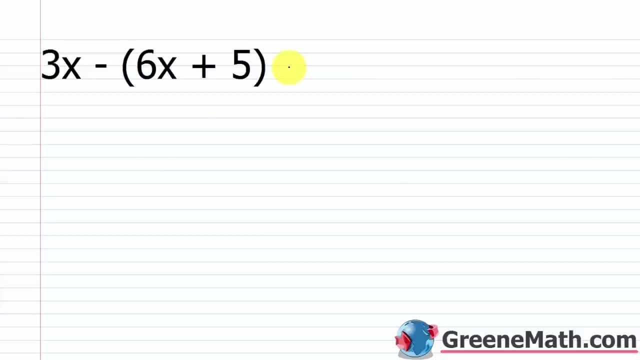 so 3x minus 6x plus 5. so again, I'm going to change this to a plus and then I can think about this as a plus negative 1. right, each sign inside the parentheses is going to change. so I'm going to have 3x plus negative. 1 times 6x is minus 6x, where I could drop the plus sign and just put. 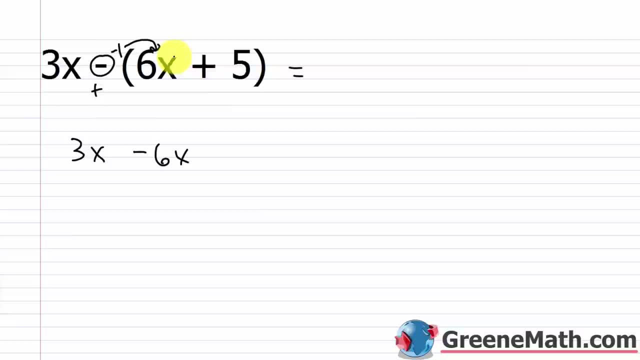 minus 6x, it doesn't matter. and then negative 1 times 5 is minus 5. 3x minus 6x is negative 3x. and then minus 5. and there's your answer: negative 3x minus 5. what about something like? 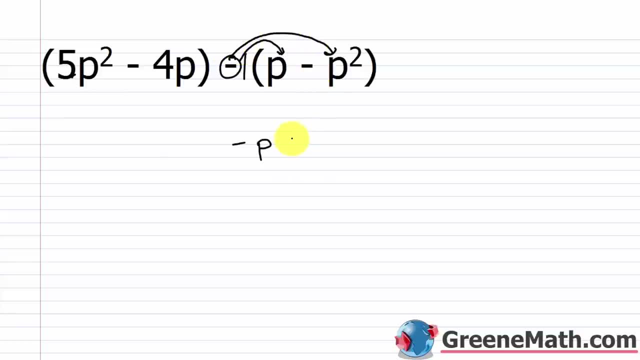 Instead of negative p squared, you're going to change the sign. This is going to be plus p squared. 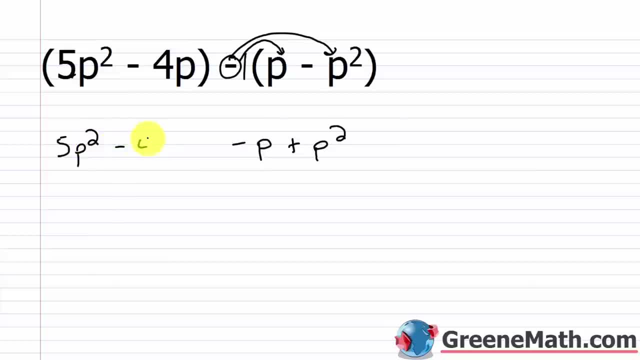 So I would have 5p squared minus 4p and then minus p plus p squared. Okay. 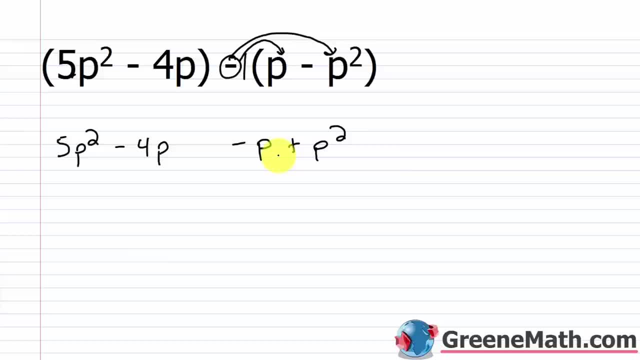 So if you're removing parentheses, you change the sign of each term inside the parentheses. 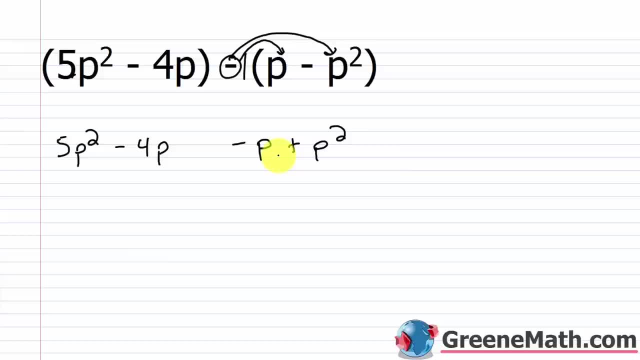 That's just the rule, whether you're working with polynomials or anything really. So now I can just set this up just like we did in the previous problems. So I have 5p squared. Plus p squared. Put my like terms next to each other. Minus 4p minus p. 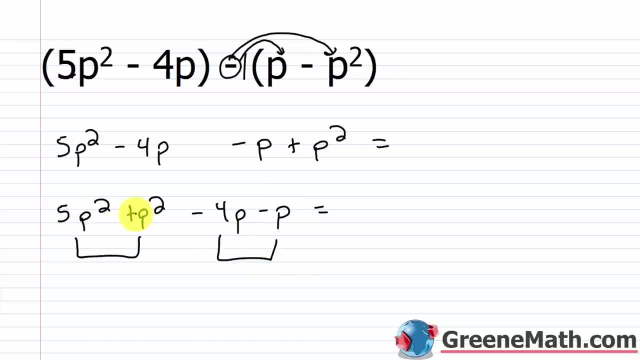 So these are like terms and these are like terms. So 5p squared plus p squared. That's going to be 6p squared. And then negative 4p minus p. That's minus 5p. There's your answer. 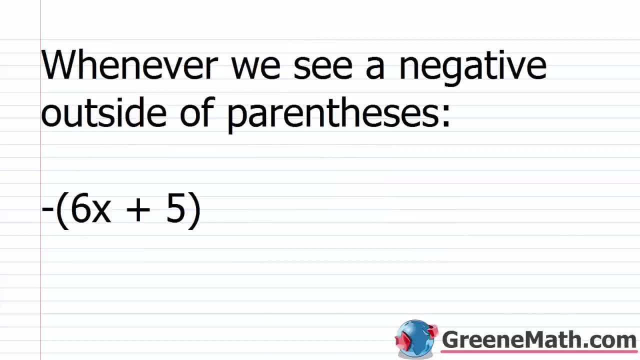 6p squared minus 5p. Again, whenever we see a negative outside of parentheses, a lot of teachers are just going to say, make this a plus negative 1 and distribute the negative 1. 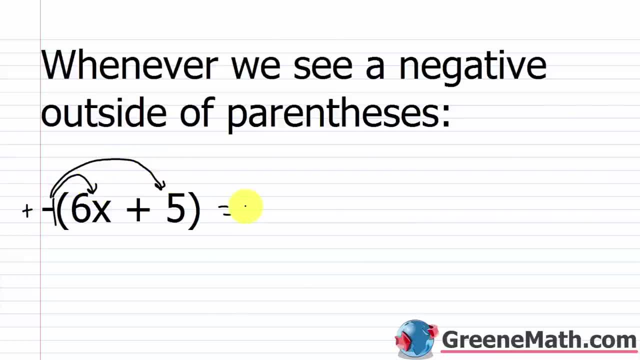 That's going to remind you to change the sign of everything. So this becomes negative 1 times 6x or negative 6x. Negative 1 times 5 or minus 5. So that's just a rule to remember just moving forward. Again, not just when you're working with polynomials, but when you're just working in math in general. Negative outside of parentheses. Change the sign of each term inside the parentheses to drop the parentheses. All right. 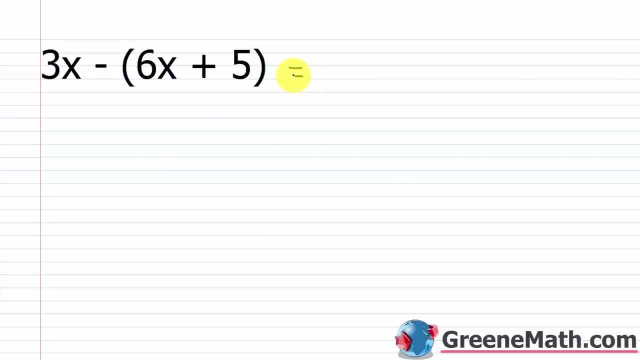 So 3x minus 6x plus 5. So again, I'm going to change this to a plus. And then I can think about this as a plus negative 1. Each sign inside the parentheses is going to change. So I'm going to have 3x plus negative 1 times 6x is minus 6x. Or I could drop the plus sign and just put minus 6x. It doesn't matter. 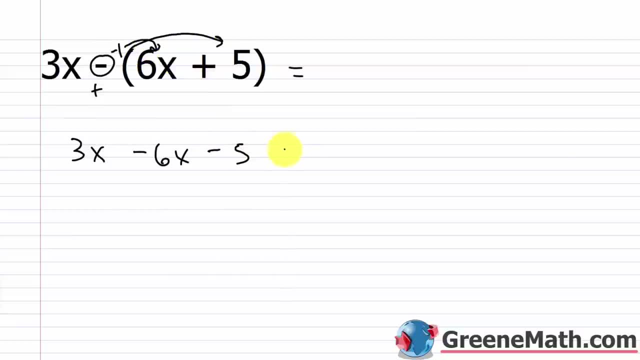 And then negative 1 times 5 is minus 5. 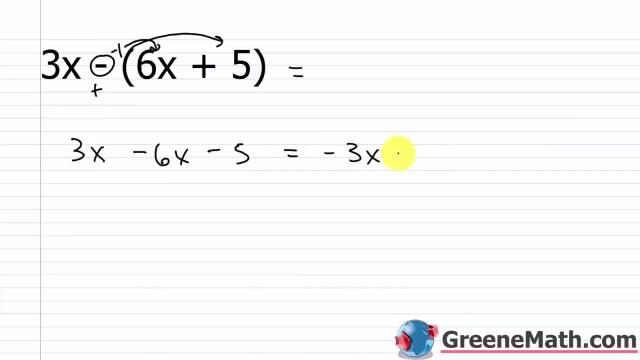 3x minus 6x is negative 3x and then minus 5. And there's your answer. Negative 3x minus 5. 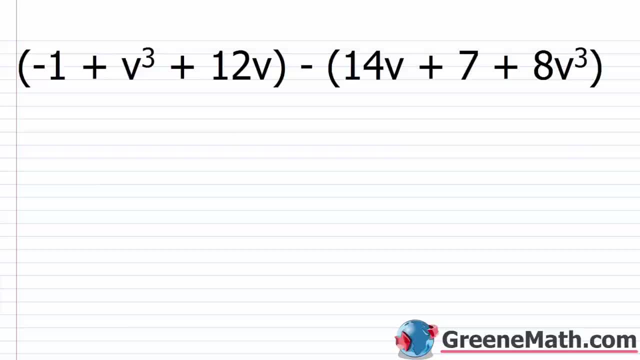 What about something like negative 1 plus v cubed plus 12v. And I'm subtracting away 14v plus 7 plus 8v cubed. 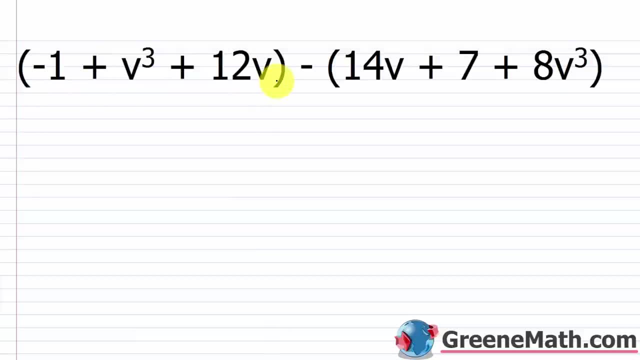 So again, this part right here, this first part stays the same. So we have negative 1 plus v cubed plus 12v. But again, if you want to save yourself a little bit of time, you can put the polynomial in standard form to start. So I could reorder this. Just kind of put the negative 1 behind everything. 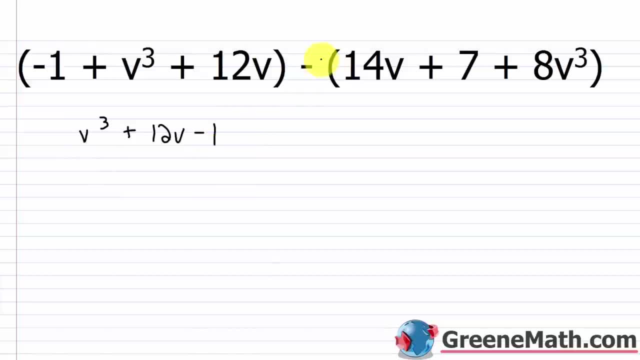 And now it's in standard form. And then I have this minus here. So what I'm going to do is I'm going to distribute. I'm going to put plus negative 1. And I'm just going to distribute the negative to each term inside the parentheses. So negative 1 times 14v is minus 14v. Negative 1 times 7 is minus 7. 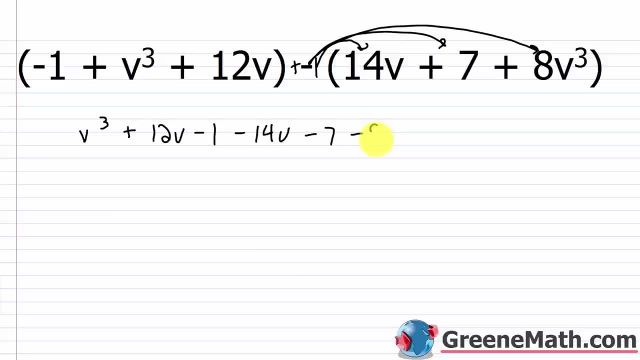 Negative 1 times 8v cubed is minus 8v cubed. Okay. So now. Again. 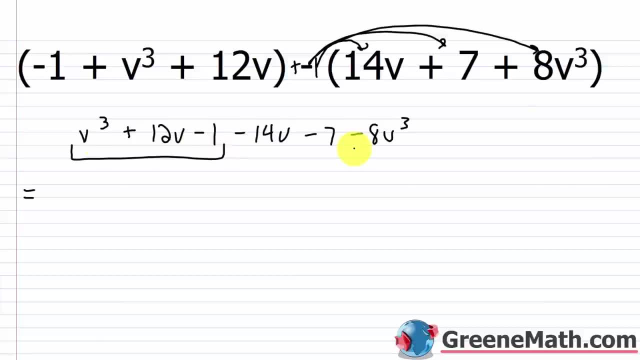 And this first polynomial, I put it in standard form. So I'm just going to follow that format. So I have v cubed minus 8v cubed. 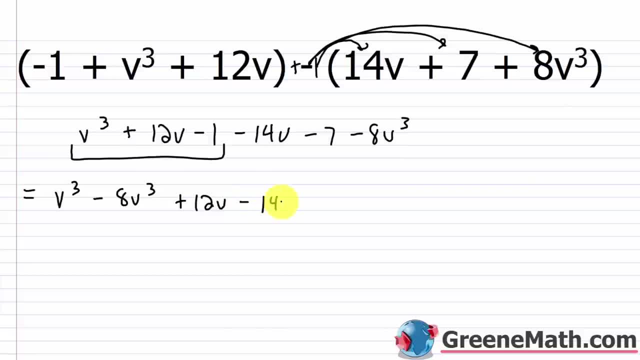 I have plus 12v minus 14v. I have minus 1 and then minus 7. 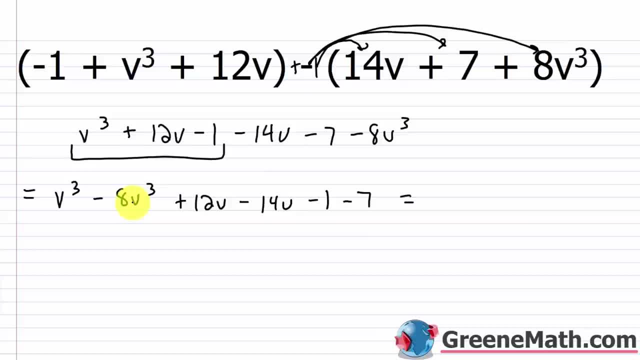 And now I just follow this. v cubed minus 8v cubed. That's going to give me negative 7v cubed. Right? 1 minus 8 is negative 7. So negative 7v cubed. And then 12v minus 14v. And that kind of looks like a u. Let me kind of make that look a little better. 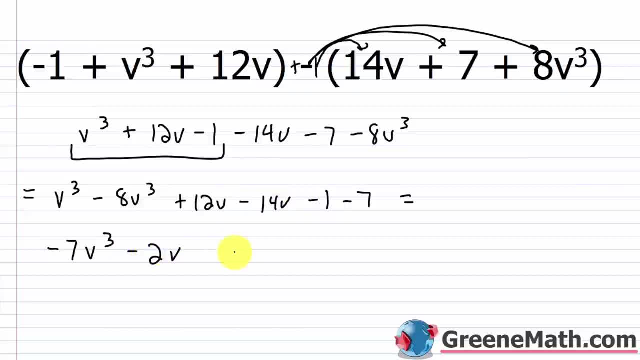 So 12v minus 14v is negative 2v. And then negative 1 minus 7 is negative 8 or minus 8. And notice how this is already in standard form for me. I have v cubed, v to the first power. And you can think of this as v to the power of 0. So it's in standard form. So negative 7v cubed minus 2v minus 8. That's your answer. 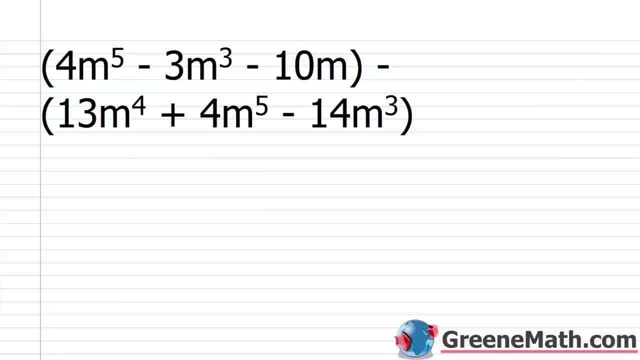 But now we're looking at 4m to the fifth power minus 3m cubed minus 10m. 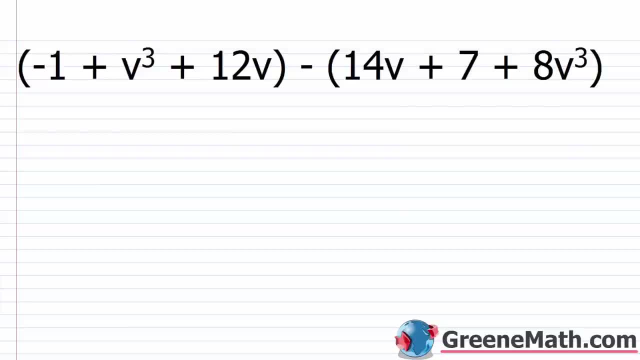 negative 1 plus v cubed plus 12v, and I'm subtracting away 14v plus 7 plus 8v cubed. so again, this part right here, this first part stays the same. so we have negative 1 plus v cubed plus 12v. but again, if you want to save yourself a little bit of time, 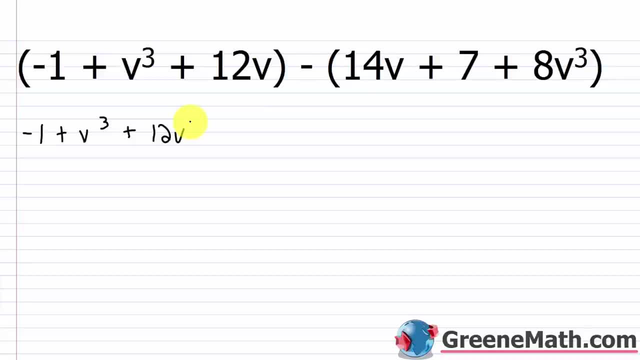 you can put the polynomial in standard form to start, so I could reorder this, just kind of put the negative 1 behind everything, and now it's in standard form, and then I have this minus here. so what I'm going to do is I'm going to distribute, I'm going to put plus negative 1 and I'm just going to distribute the negative. 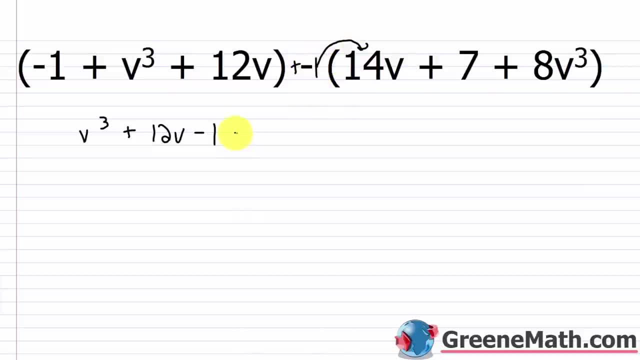 to each term inside the parentheses. so: negative 1 times 14v is minus 14v. negative 1 times 7 is minus 7. negative 1 times 8v cubed is minus 8v cubed. okay, you can see that I'm going to put this in standard form and then I'm going to put this in standard form. 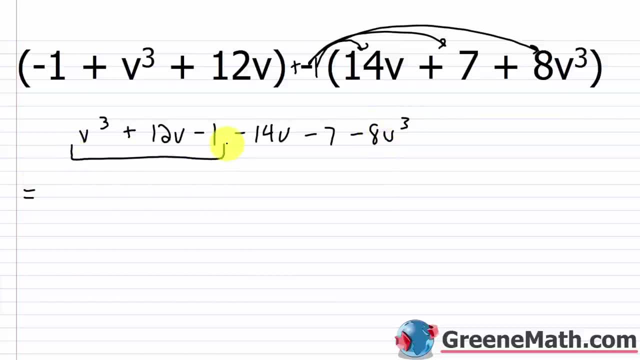 so now again this first polynomial. I put it in standard form, so I'm just going to follow that format. so I have v cubed minus 8v cubed, I have plus 12v, minus 14v, I have minus 1 and then minus 7. 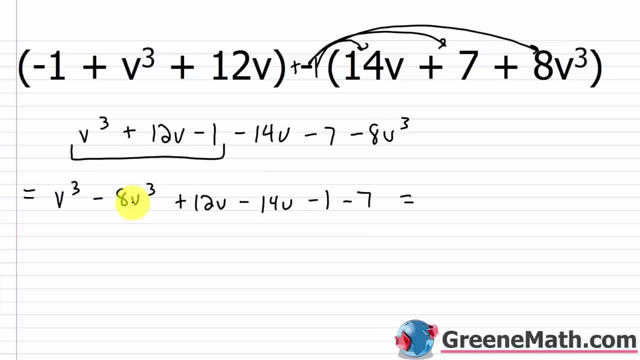 and now I just follow this: v cubed minus 8v cubed, that's going to give me negative 7v cubed right. 1 minus 8 is negative 7, so negative 7v cubed. and then 12v minus 14v is minus 7v cubed. 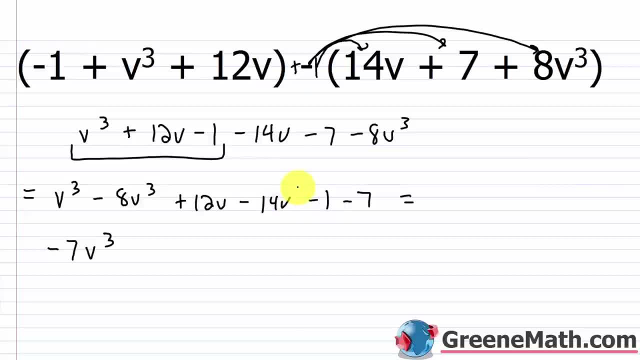 and that kind of looks like a? u let me kind of make that look a little better. so 12v minus 14v is negative 2v, and then negative 1 minus 7 is negative 8 or minus 8, and notice how this is already in. 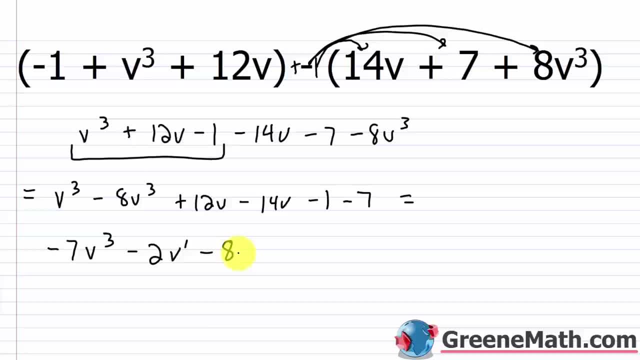 standard form for me. I have v cubed, v to the first power and you can think of this as v to the power of 0. so it's in standard form so negative 7v cubed minus 2v minus 8. that's your answer. 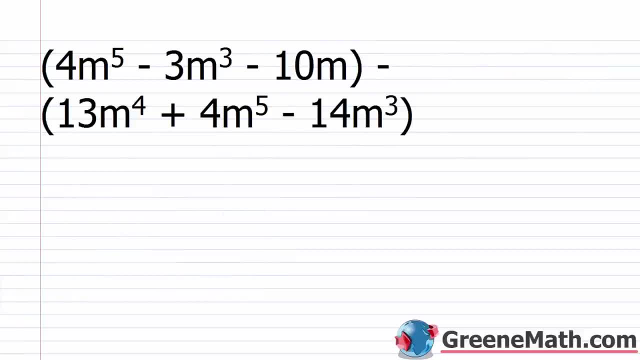 all right. now we're looking at 4 and we're going to put this in standard form. so negative 7v cubed minus 4m to the fifth. power minus 3m cubed minus 10m and we're subtracting away 13m to the fourth. 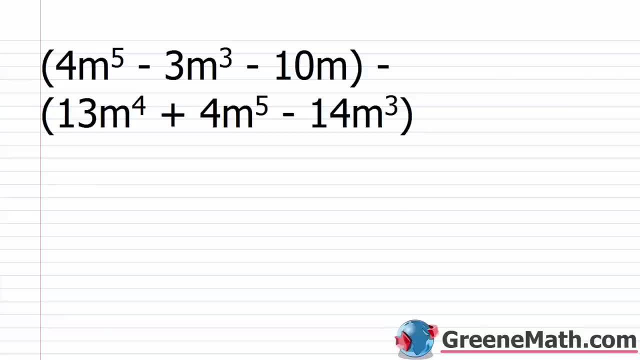 And we're subtracting away 13m to the fourth power plus 4m to the fifth power minus 14m cubed. 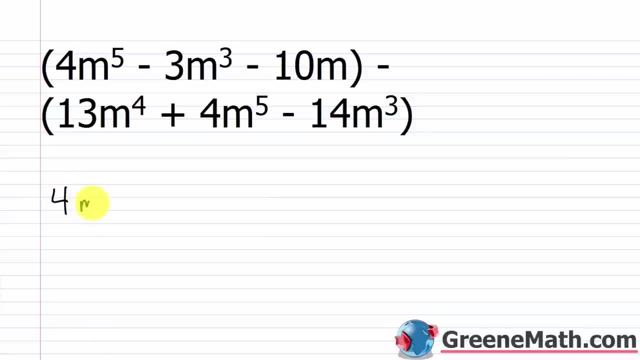 So again, this first part stays the same. So I have 4m to the fifth power minus 3m cubed minus 10m. And then, look, I have this minus sign that's out in front of the parentheses. So just put plus negative 1. I know this is kind of off down to the next line. So let me put the negative 1 over here actually. Make it a little easier to see. So the negative 1, we multiply this by 13m to the fourth power. 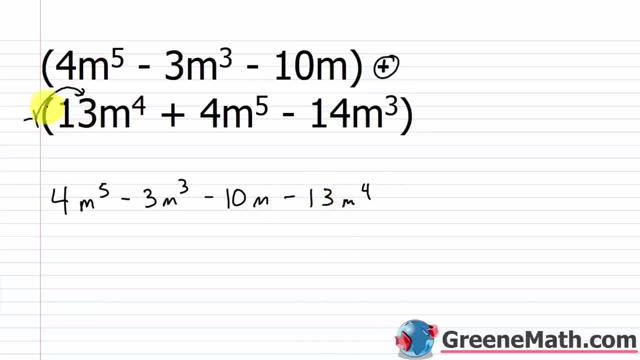 So minus 13m to the fourth power. And we multiply it by 4m to the fifth power. So minus 4m to the fifth power. And lastly, we multiply it by negative 14m cubed. 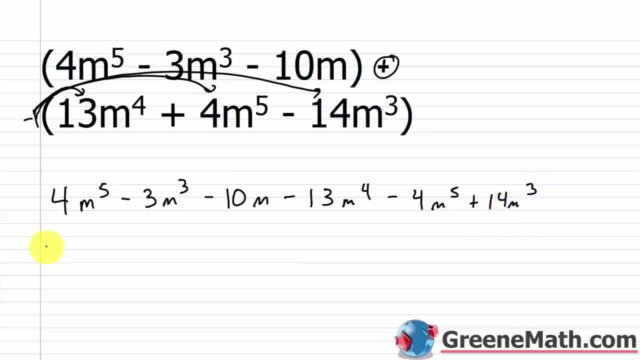 So plus 14m cubed. All right. 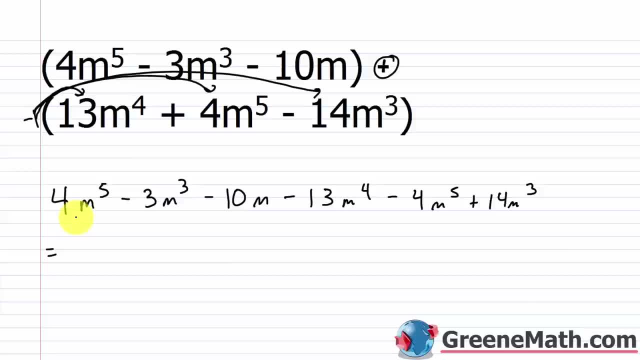 So if I look at this, I can kind of combine like terms here. I don't need to write everything next to each other. That's going to save you a little time. 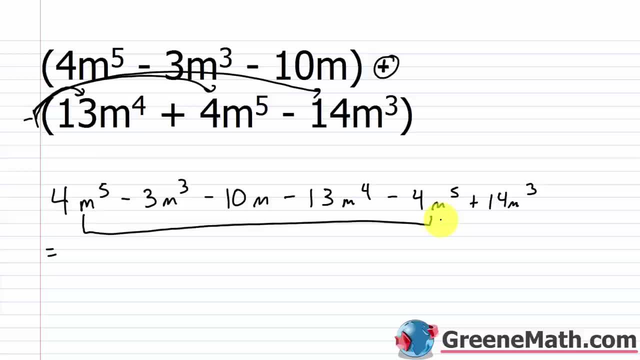 So 4m to the fifth power and negative 4m to the fifth power, those are going to cancel. All right. 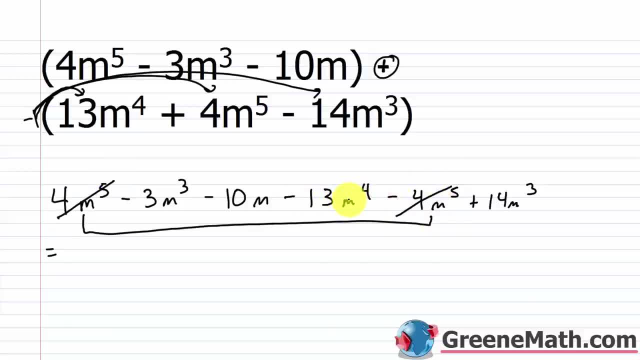 Those are opposites. Next, I'm going to look at this negative 13m to the fourth power. 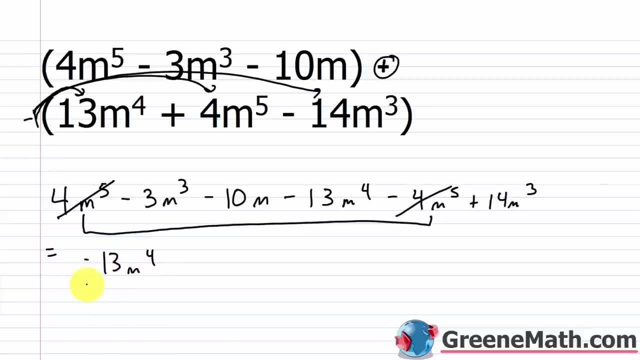 Negative 13m to the fourth power. There's no like terms to combine with this. So we're just going to leave this out in front. That's going to be my term that has the highest degree. So it's going to go first. 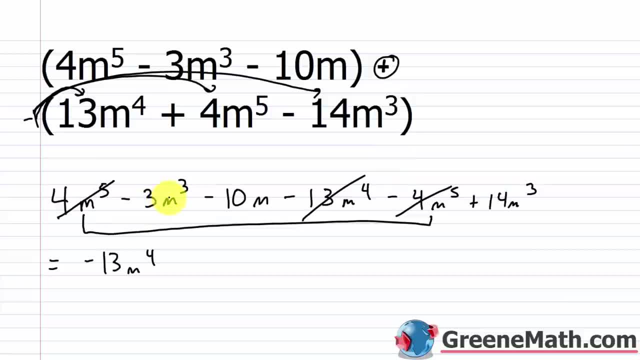 And I can cross it out as I use it. And then I have negative 3m cubed. And 14m cubed. Negative 3 plus 14 is 11. So this is going to be plus 11m cubed. Cross it out as I use it. 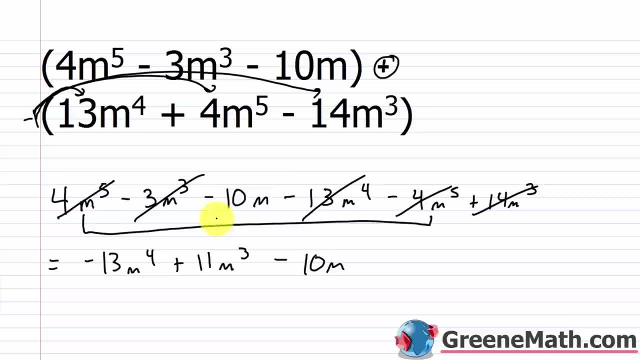 And then minus 10m. And again, these little tricks that I give you for, you know, crossing stuff out and using that, these are things that a lot of people use just so that they don't get confused. 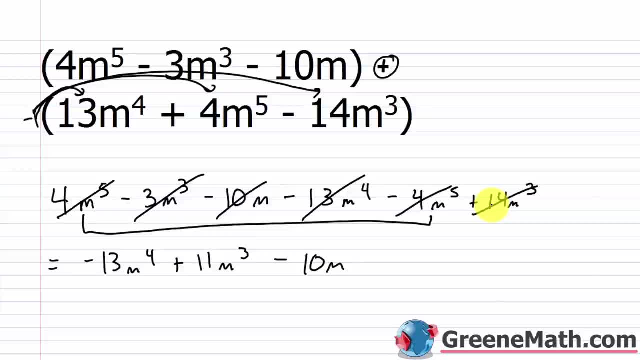 A lot of these problems start getting longer and longer and more tedious. And you need some kind of way to just keep track of what you've worked on and what you haven't. All right. So that you get the right answer. 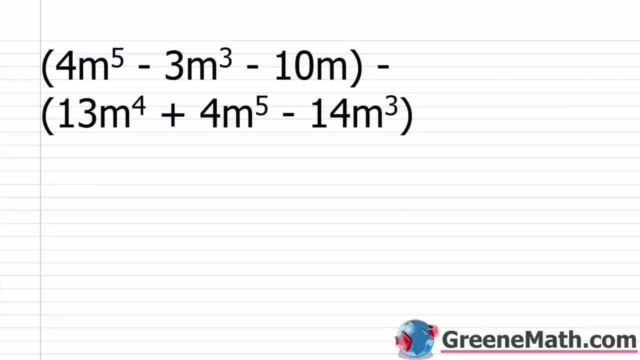 power plus 4m to the fifth power minus 14m cubed. so again, this first part stays the same. so I have 4m to the fifth power minus 3m cubed, minus 10m, and then look, I have this minus sign. that's out. 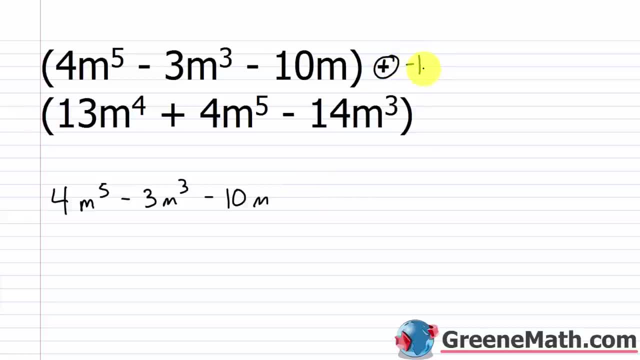 in front of the parentheses. so just put plus negative 1 and I know this is kind of off down to the next one, but I'm going to put it in standard form. so I'm going to put it in standard form, next line. so let me put the negative 1 over here. actually make it a little easier to see. 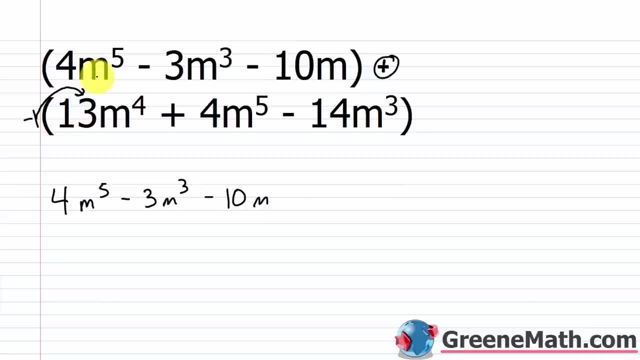 so the negative 1. we multiply this by 13m to the fourth power, so minus 13m to the fourth power. and we multiply it by 4m to the fifth power, so minus 4m to the fifth power. then, lastly, we multiply it by negative 14m cubed, so plus 14m cubed. all right. so if I look at this, I can kind 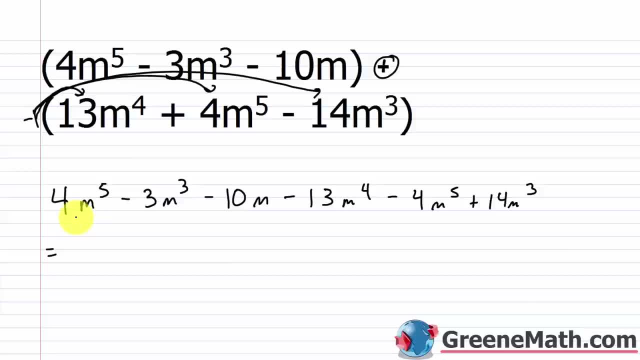 of combine like terms here. I don't need to write everything next to each other. that's going to save you a little time. so I'm going to write everything next to each other and I'm going to write everything. so 4m to the fifth power and negative 4m to the fifth power, those are going to cancel, right those? 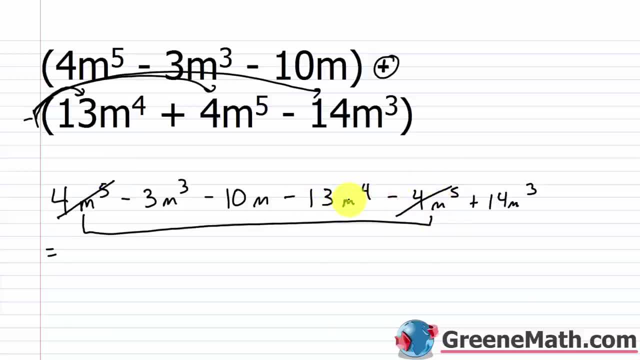 are opposites. next I'm going to look at this: negative 13m to the fourth power. negative 13m to the fourth power. there's no like terms to combine with this, so we're just going to leave this out in front. that's going to be my term, that has the highest degree, so it's going to go first. 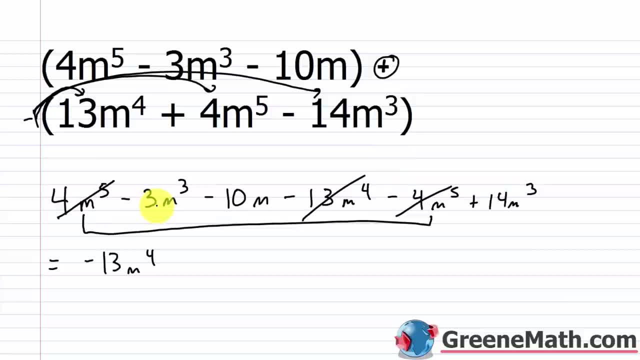 and I can cross it out as I use it. and then I have negative 3m cubed and 14m cubed. negative 3 plus 14 is equal to negative 3m cubed and 14m cubed is equal to negative 3m cubed and 14m cubed is equal to. 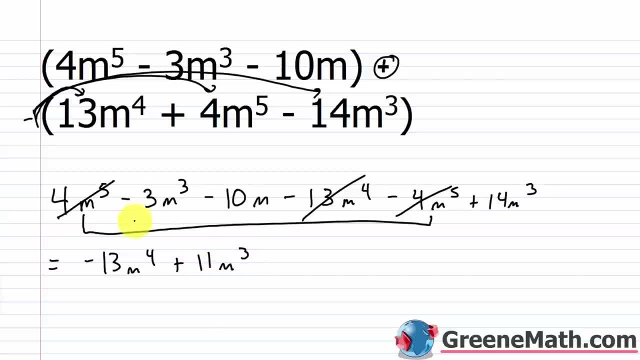 11. so this is going to be plus 11m- cubed- cross it out as you use it- and then minus 10m, and again these little tricks that I give you, for you know, crossing stuff out and using that. these are things that a lot of people use, just so that they don't get confused. 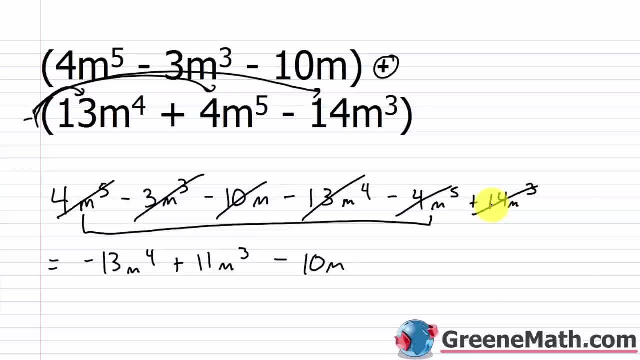 a lot of these problems start getting longer and longer and more tedious, and you need some kind of way to just keep track of what you've worked on and what you haven't right, so that you get the right answer, because the last thing you want to do is completely understand something and just make 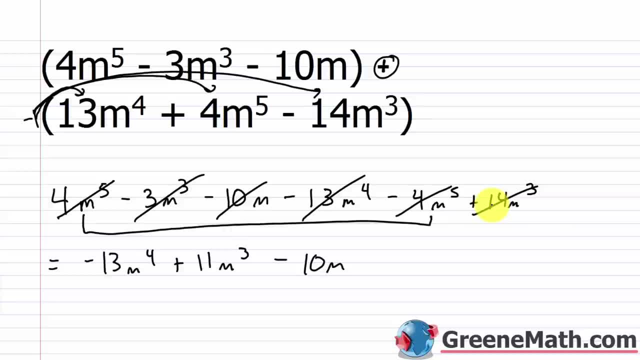 Because the last thing you want to do is completely understand something. And just make some silly error. And, you know, not get 100 on your test. All right. You want to get the highest grade possible. 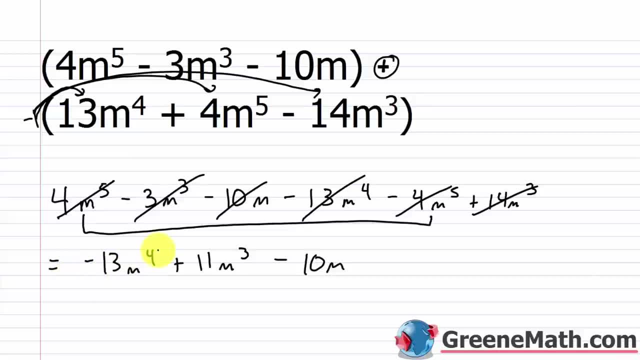 So we're going to end up with a result here of negative 13m to the fourth power plus 11m cubed minus 10m. 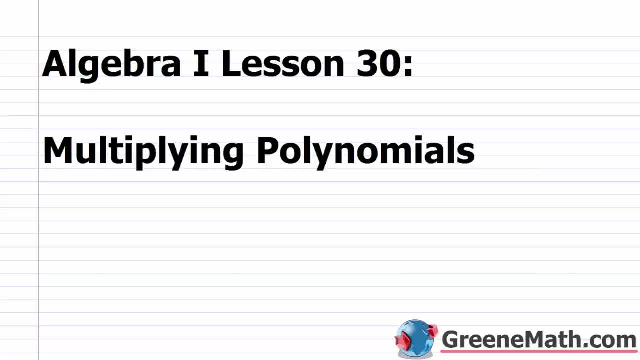 Hello and welcome to Algebra 1 Lesson 30. In this video, we're going to learn about multiplying polynomials. 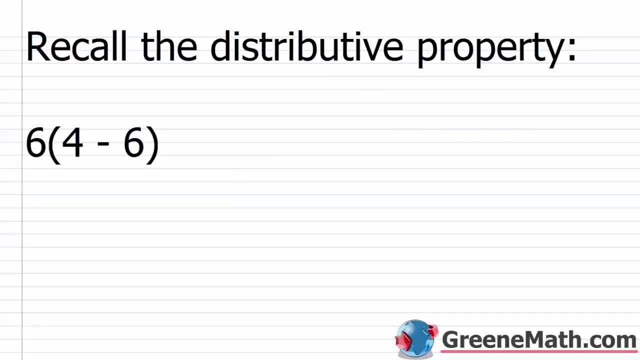 So before we jump in and start talking about multiplying polynomials, I want everybody to recall the distributive property. So have something like 6 times the quantity 4 minus 6. Remember, I can remove the parentheses here and write this as 6 times 4. 6 times 4 minus 6 times 6. So 6 times 4 is 24 minus 6 times 6, which is 36. 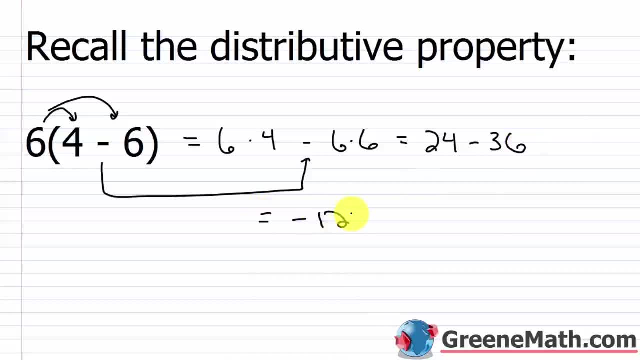 And this gives me a result of negative 12. And I can see that by just working inside the parentheses first. If I had done 4 minus 6, that would give me negative 2. And then I would have 6 times negative 2, which would also give me negative 12. 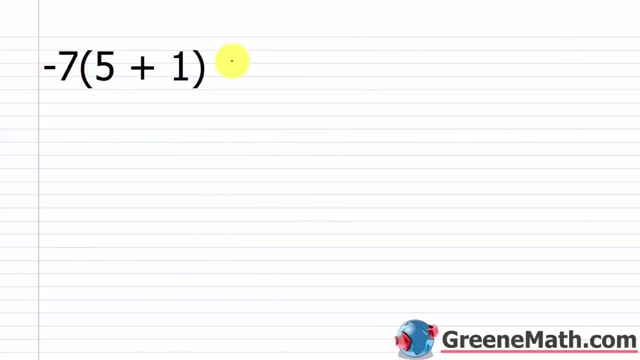 As another example, if I have negative 7 times the quantity 5 plus 1. Again, I can remove the parentheses by multiplying negative 7 times 5. Negative 7 times 5 plus negative 7 times 1. Negative 7 times 1. So negative 7 times 5 is negative 5. 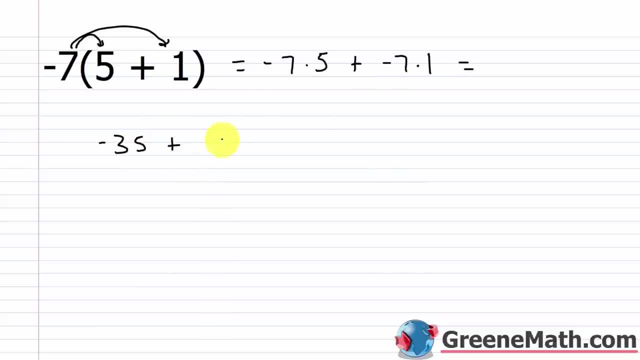 Negative 35 plus negative 7 times 1. That's negative 7. And this gives me negative 42. 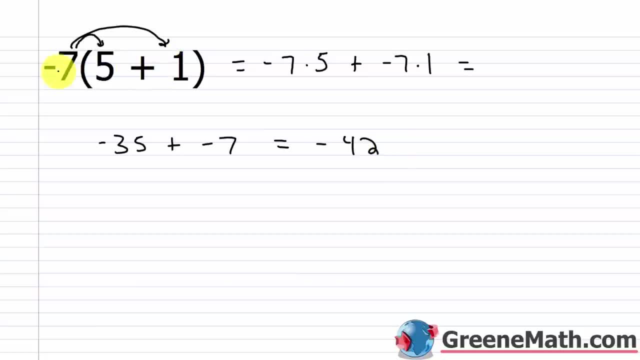 Again, I could have found the same thing by just saying, OK, 5 plus 1 is 6. Negative 7 times 6 is negative 42. 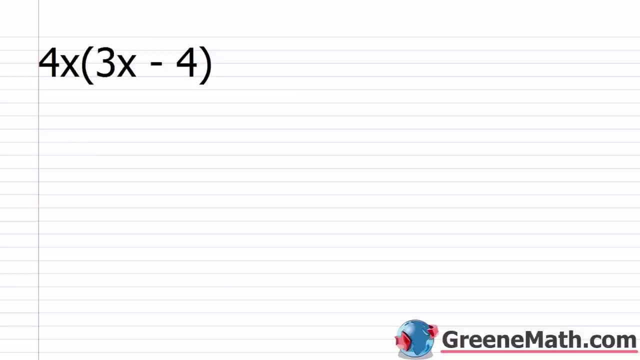 So at this point, we should be very familiar with the distributive property since we've been using it all throughout Algebra 1 and most of pre-algebra. So now we're going to use the same technique to multiply a monomial. 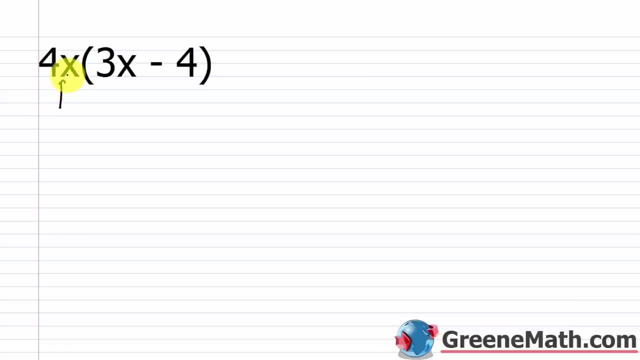 That's a polynomial that has just one single term. This is a polynomial with two terms. 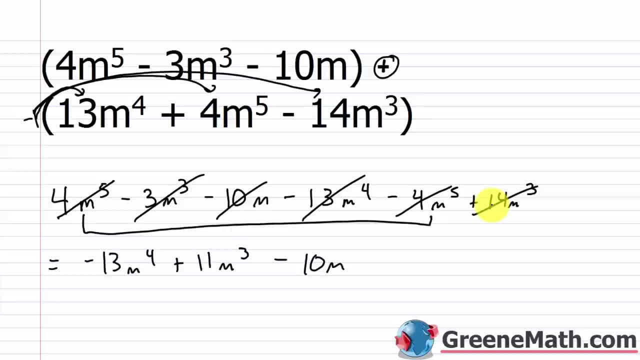 some kind of way to just keep track of what you've worked on and what you haven't right, so that you some silly error and you know not get 100 on your test right. you want to get the highest grade possible, so we're going to end up with a result here of negative 13m to the fourth power plus 11m. 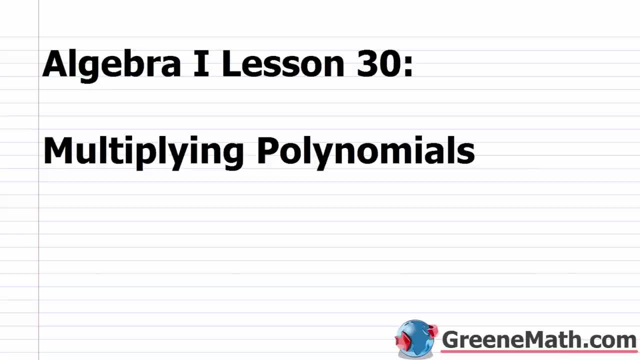 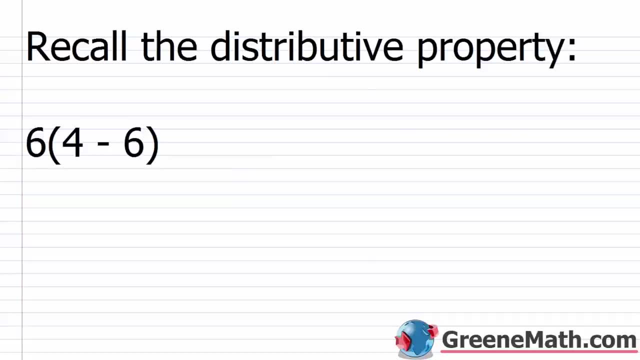 cubed minus 10m. hello and welcome to algebra 1, lesson 30. in this video we're going to learn about multiplying polynomials. so before we jump in and start talking about multiplying polynomials, want everybody to recall the distributive property. so have something like 6 times the quantity 4 minus. 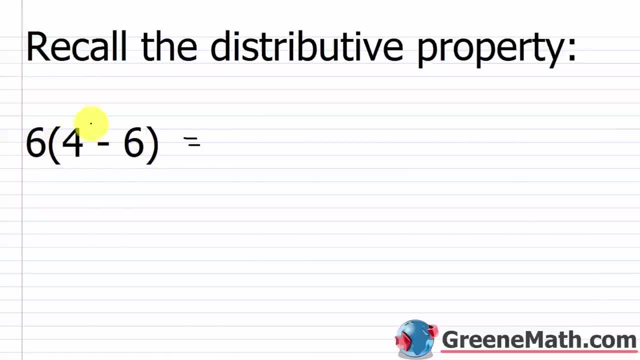 6. remember i can remove the parentheses here and write this as 6 times 4, 6 times 4 minus a minus 6 times 6.. so 6 times 4 is 24 minus 6 times 6, which is 36, and this gives me a result of negative 12.. 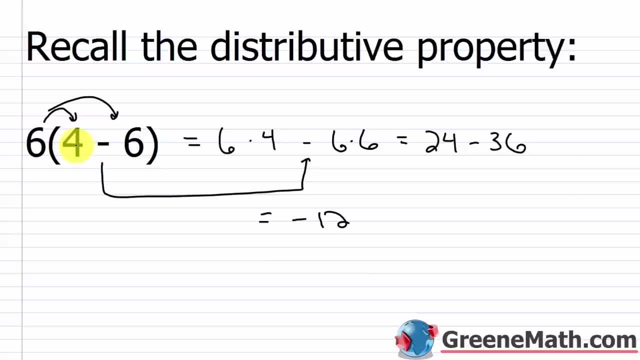 and i can see that by just working inside the parentheses. first, if i had done 4 minus 6, that would give me negative 2, and then i would have 6 times negative 2, which would also give me negative 12.. as another example, if i have negative 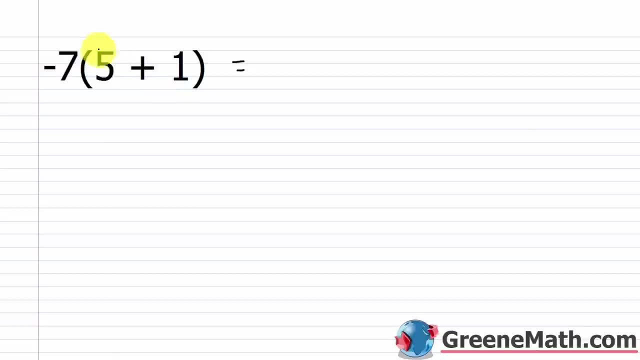 7 times the quantity 5 plus 1. again i can remove the parentheses by multiplying: negative 7 times 5, negative 7 times 5, plus negative 7 times 1. negative 7 times 1.. so negative 7 times 5 is negative 35. 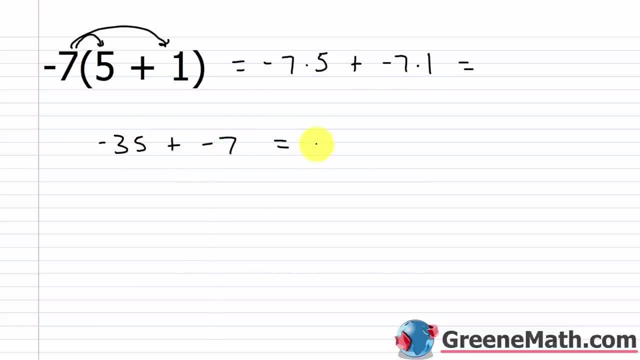 plus negative 7 times 1, that's negative 7 and this gives me negative 42.. again, i could have found the same thing by just saying: okay, 5 plus 1 is 6 negative. 7 times 6 is negative 42.. so at this, 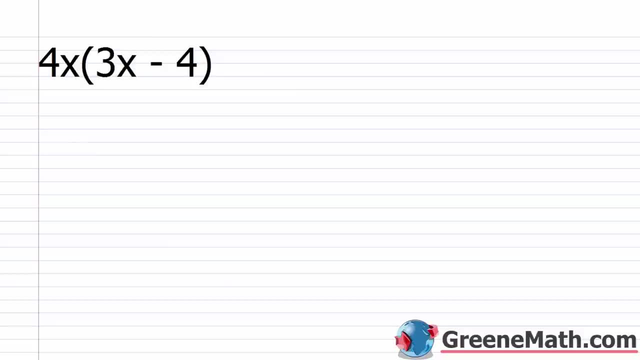 point. we should be very familiar with the distributive property, since we've been using it all throughout algebra 1 and most of pre-algebra. so now we're going to use the same technique to multiply a monomial right, that's a polynomial that has just one single term. 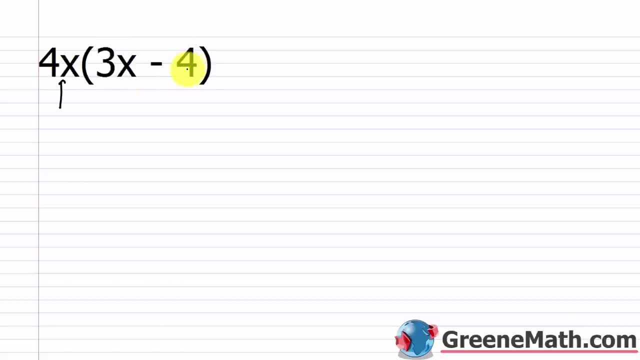 times a binomial right. this is a polynomial with two terms. so we're going to have 4x times the quantity 3x minus four, 4x times the quantity 3x minus 4.. So how are we gonna do this? 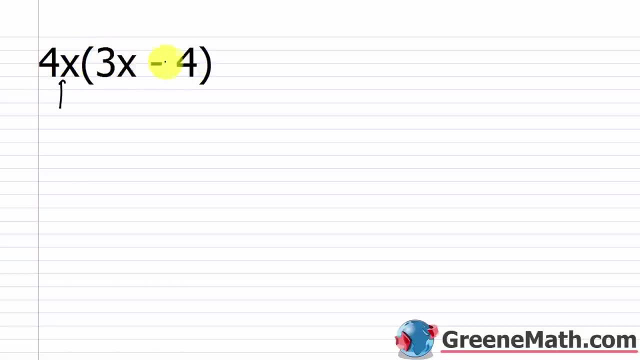 So we're going to have 4x times the quantity 3x minus 4. So how are we going to do this? We're going to use the distributive property. Remember, I'm going to take this guy out here, and I'm going to multiply it by each term inside the parentheses. 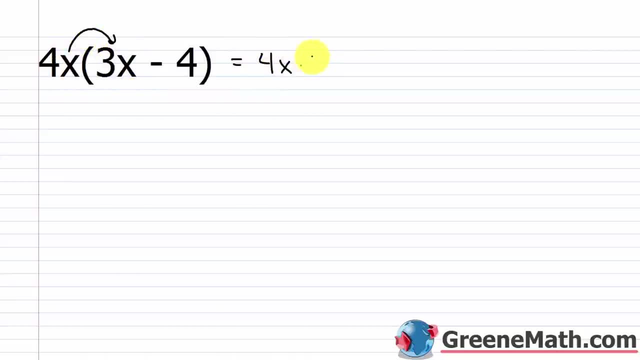 So 4x times 3x. And then I have that minus there. 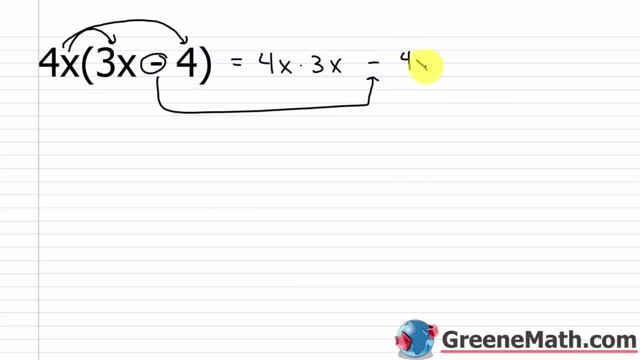 And then we have 4x times 4. So for something like 4x times 3x, how do we do that? 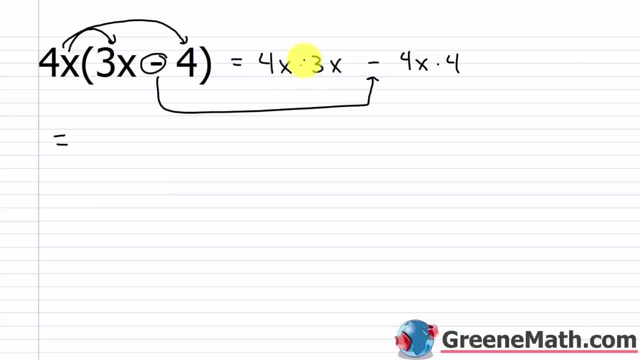 Well, you'd multiply the number parts together, the coefficients. What is 4 times 3? Well, that's going to be 12. Then you'd multiply the variables together. So I have x times x. So I know from my rules of exponents that if I'm multiplying and I have the same base, I would just add the exponents. 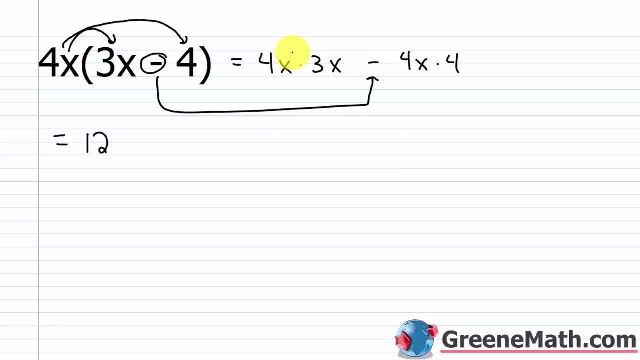 I keep the base the same, add the exponents. So this has an exponent of 1, and so does this. So x times x is x raised to the second power, 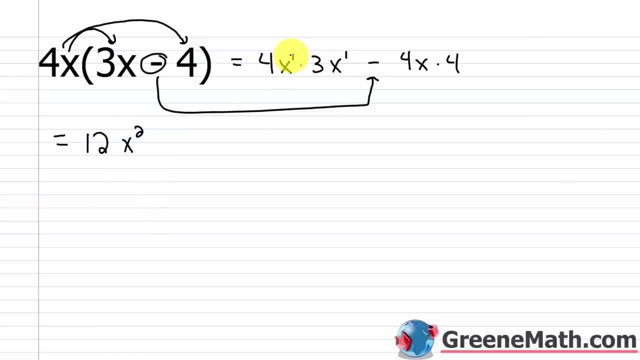 or x squared. Keep the base the same, so x stays the same. And then add 1 plus 1, that's 2. 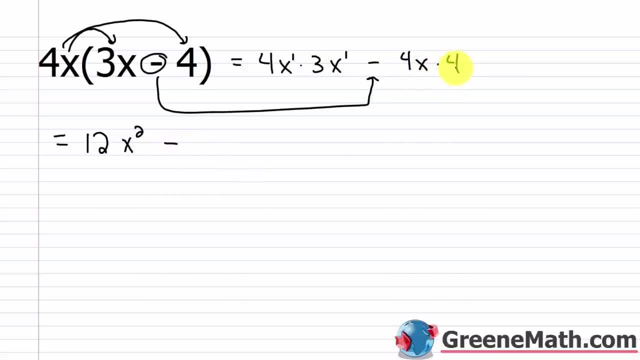 Then we're subtracting away. Now we have 4x times 4. 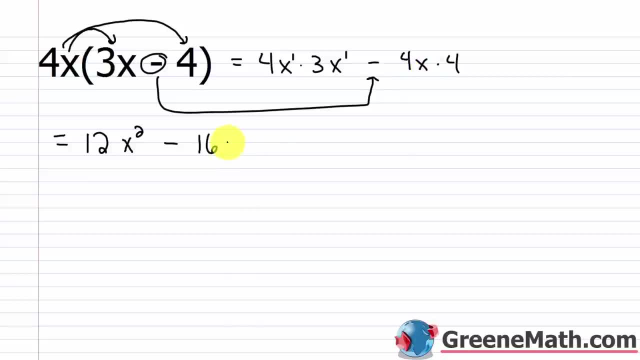 So 4 times 4 is 16. And then x just comes along for the ride. So that's 16x. 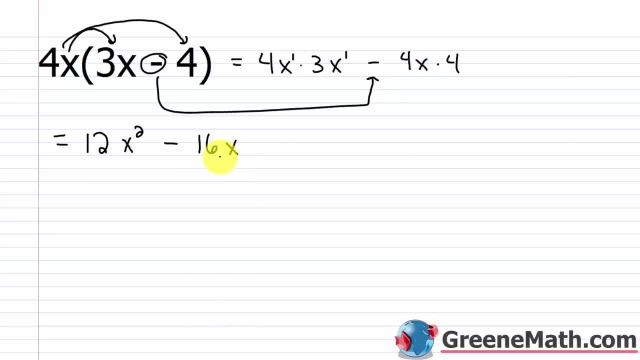 So we end up with 12x squared minus 16x. 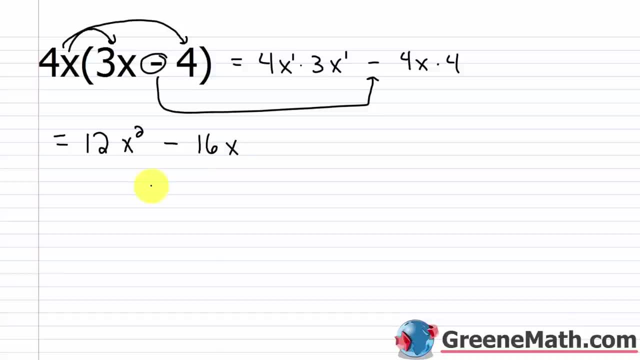 And when you're working with polynomials, you always want to make sure that you don't have any more like terms that you can combine. I have an x squared here, and I have an x here. Those are not like terms, so this is the best that we can do. All right, for the next one, 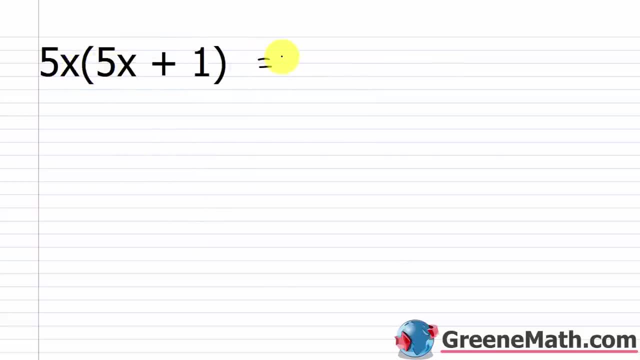 I have 5x times the quantity 5x plus 1. And again, I'm just going to use my distributive property. So 5x times 5x. 5x times 5x. And then plus. Next I'm going to have 5x times 1. 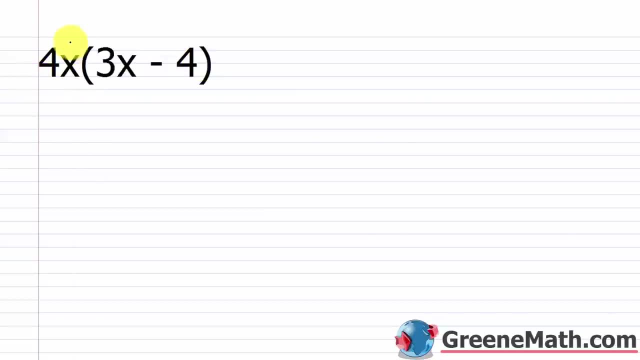 We're gonna use the distributive property. Remember, I'm gonna take this guy out here and I'm gonna multiply it by each term inside the parentheses. So four x times three x, and then I have that minus there, and then we have four x times four. 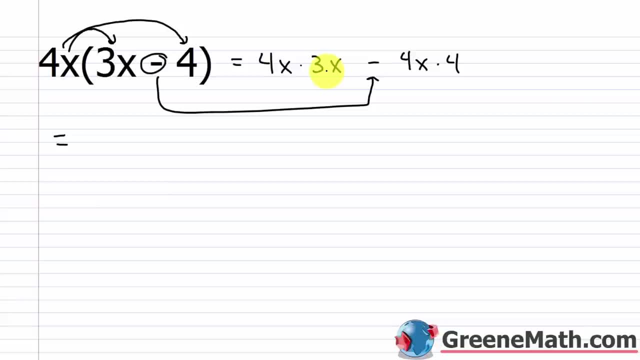 So for something like four x times three x. how do we do that? Well, you'd multiply the number parts together, the coefficients, right? What is four times three? Well, that's gonna be 12.. Then you'd multiply the variables together. 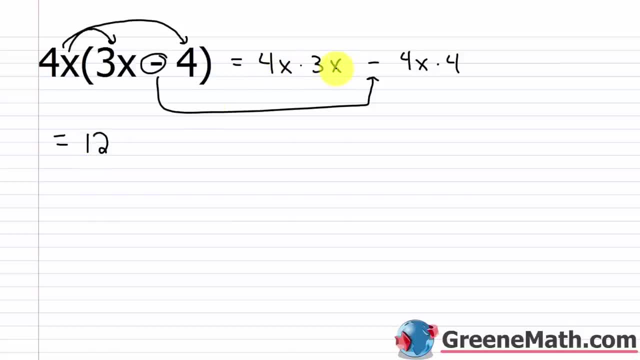 So I have x times x. So I know from my rules of exponents that if I'm multiplying and I have the same base, I would just add the exponents. right, I keep the base the same, add the exponents. So this has an exponent of one, and so does this. 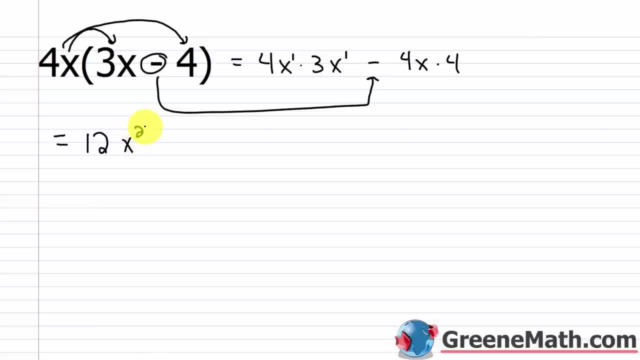 So x times x is x raised to the second power or x squared right. Keep the base the same, so x stays the same, and then add one plus one, that's two. All right, then we're subtracting away. 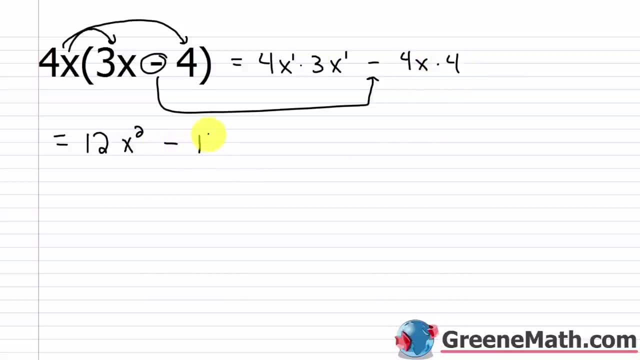 Now we have four x times four, So four times four is 16, and then x just comes along for the ride, So that's 16 x. So we end up with 12 x squared minus 16 x. And when you're working with polynomials, 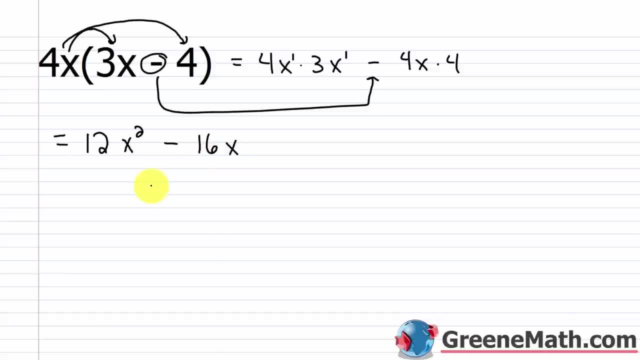 you always wanna make sure that you don't have any more like terms that you can combine. I have an x squared here and I have an x here. Those are not like terms, So this is the best that we can do: 12 x squared minus 16 x. 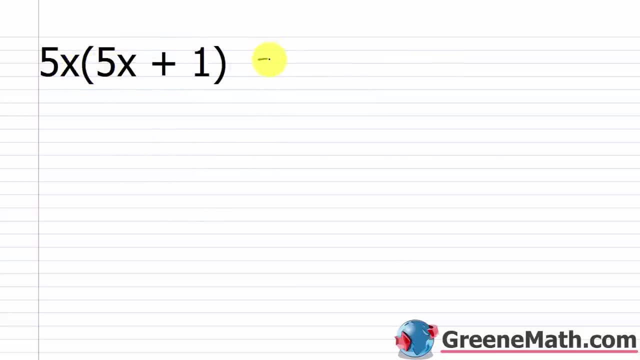 All right, for the next one I have five x times the quantity, five x plus one, And again I'm just gonna use my distributive property. So five x times five x, Five x times five x And then plus. Next I'm gonna have five x times one. 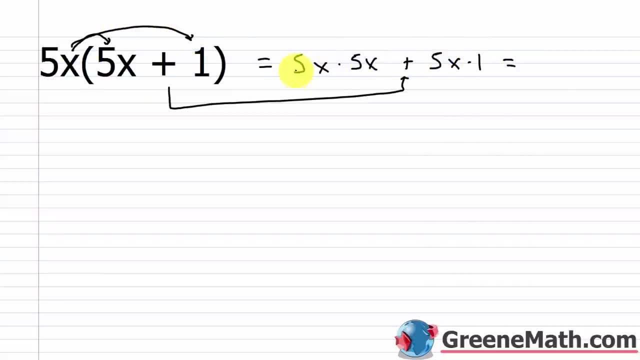 Five x times one. So five x times five x, five times five is 25.. And then x times x again is x squared. And then plus Five x times one is five x. So these two are not like terms, right. 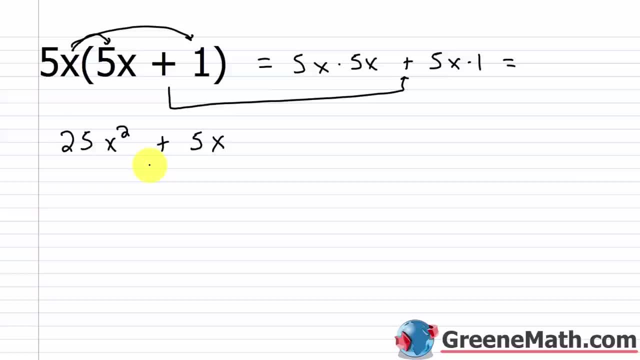 You have x squared and you have x. So that's gonna be our answer: 25 x squared plus five x. What about something like three p times the quantity four p plus two? Again, I'm gonna use my distributive property. So three p times four p. 5x times 1. So 5x times 5x. 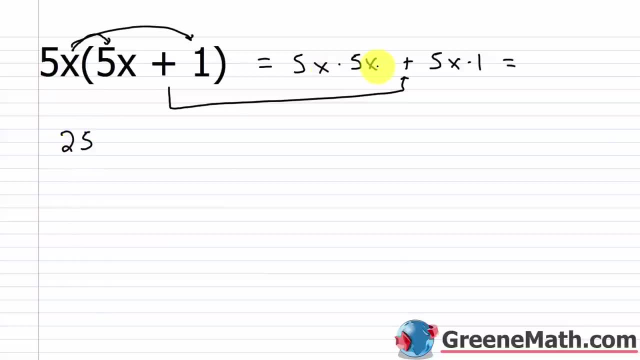 5 times 5 is 25. And then x times x, again, is x squared. 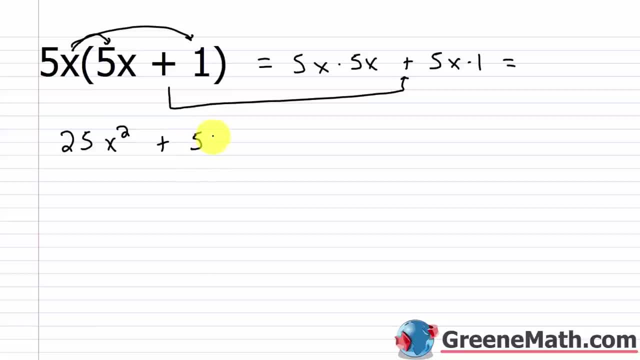 And then plus 5x times 1 is 5x. So these two are not like terms, right? You have x squared and you have x. So that's going to be our answer. 25x squared plus 5x. 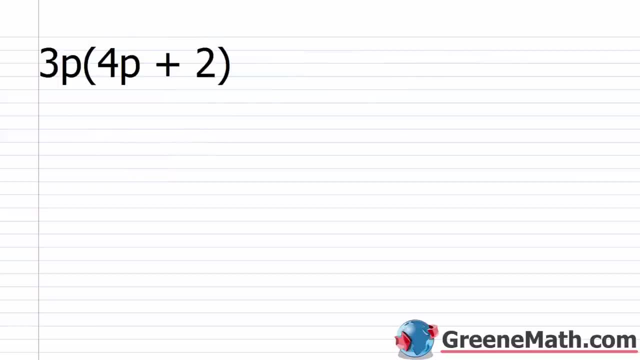 What about something like 3p times the quantity 4p plus 2? Again, I'm going to use my distributive property. So 3p times 4p. 3p times 4p. Plus, right, this guy's going to go over there. 3p times 2. 3p times 2. So 3p times 4p. 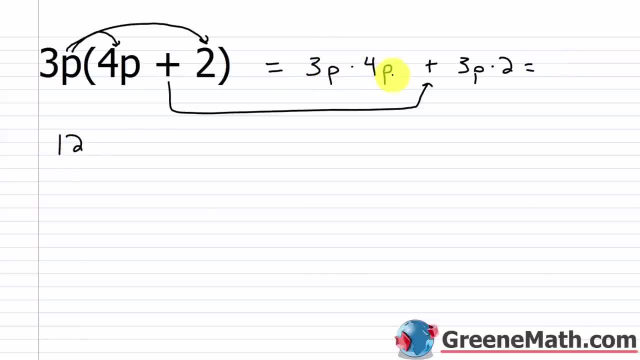 You do 3 times 4, that's 12. And then p times p is p squared. Then plus. Next we have 3p times 2. 2 times 3 is 6. And then p just comes along for the ride. So that's 6p. So I end up with 12p squared plus 6p as my answer. All right. 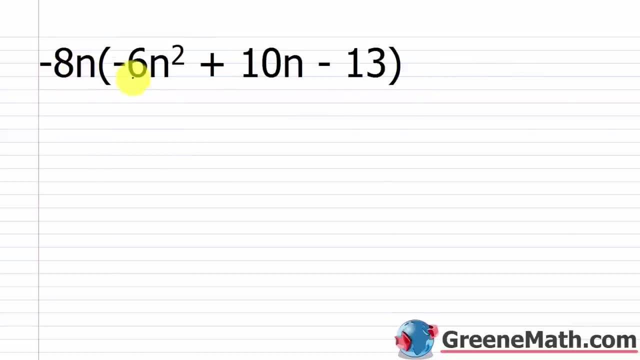 Now I'm going to make it a little bit more tedious. We have a monomial that's being multiplied by a trinomial. And a trinomial is just a polynomial with three terms. 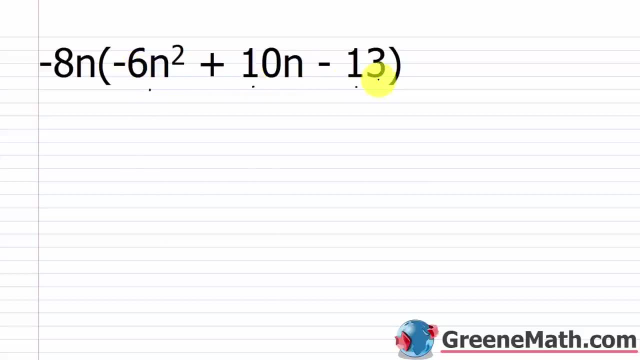 You have one, two, three terms. Same principle here. 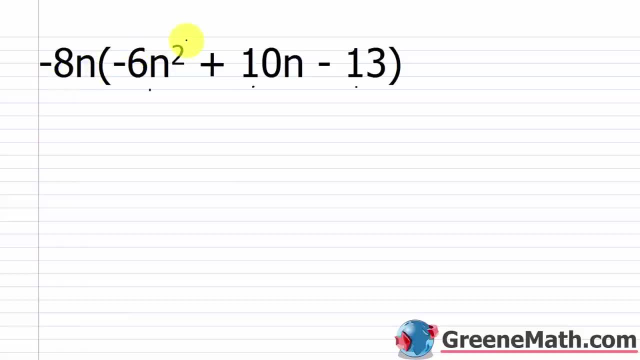 I'm going to take this guy right here, multiply by each term inside the parentheses. So we have negative 8n times this quantity, negative 6n squared plus 10n minus 13. And I'm just going to say, okay, negative 8n times negative 6n squared. So negative 8n times negative 6n squared. 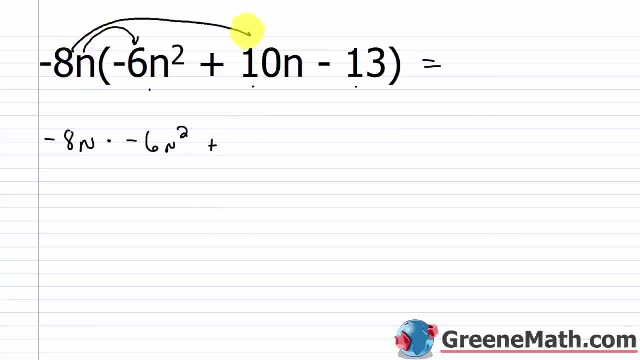 Then plus. I'll have negative 8n times 10n. And then minus. Minus. 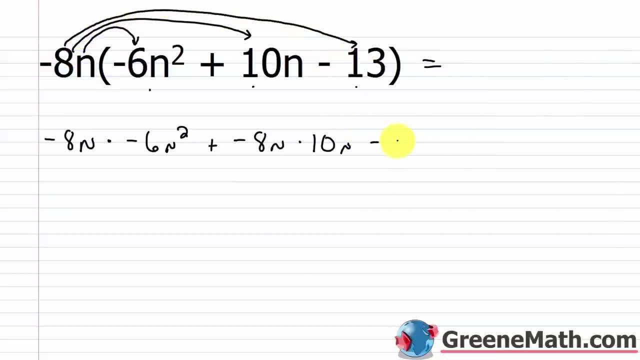 I have negative 8n times 13. 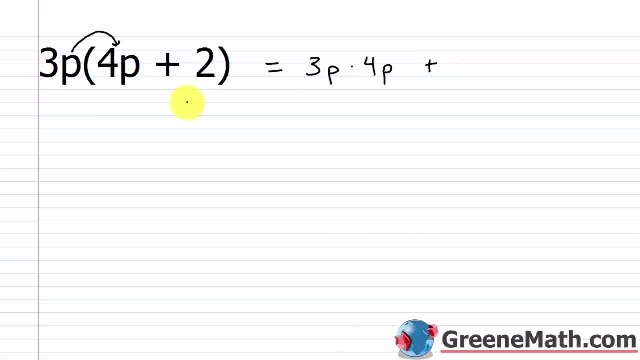 Three p times four, p Plus. all right, this guy's gonna go over there. Three p times two, Three p times two, So three p times four p. You do three times four, that's 12.. And then p times p is p squared. 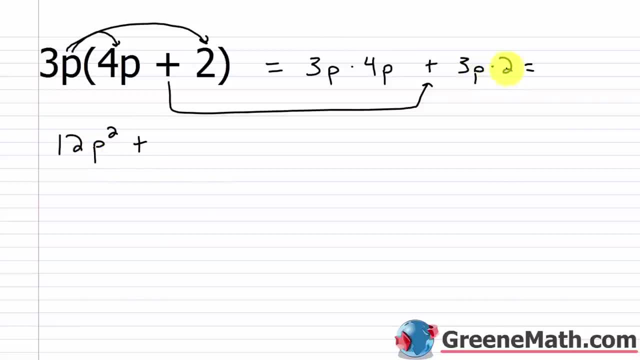 Then plus Next, we have three p times two. Two times three is six, And then p just comes along for the ride, So that's six p. So I end up with 12 p squared plus six p as my answer. All right, now I'm gonna make it a little bit more tedious. 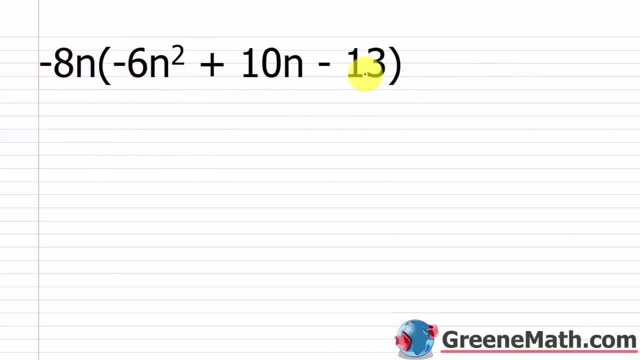 We have a monomial that's being multiplied by a trinomial, And a trinomial is just a polynomial with three terms. You have one, two, three terms. Same principle here. I'm gonna take this guy right here: multiply by each term inside the parentheses. 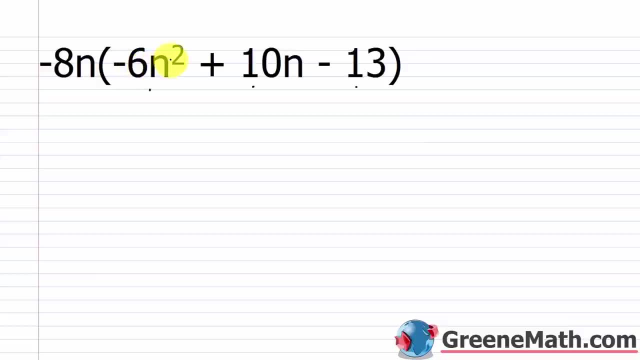 So we have negative eight n times this quantity, negative six n squared, plus 10 n, minus 13.. And I'm just gonna say, okay, negative eight n times negative six n squared. So negative eight n times negative six n squared. Then plus, I'll have negative eight n times 10 n. 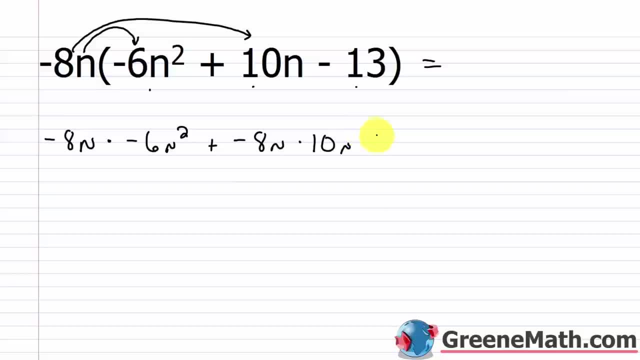 So negative eight n times 10 n, And then minus, minus, I have a negative eight n times 13.. And one of the things you can do here, you can think about this as negative 13,. right, So you don't make a sign mistake. 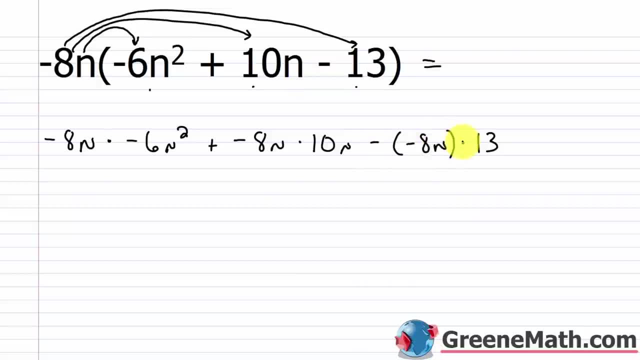 Or you can have a minus, so you'd end up with minus and negative. We know that would be plus a positive, But just to make this easy on us, I'm just gonna put plus right here And I'm gonna write this as a negative 13.. 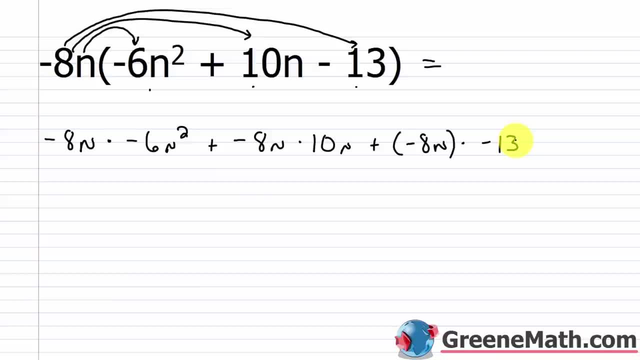 Okay, so let's go through and crank out the multiplication. So: negative eight n times negative, six n squared Negative eight times negative: six is first off a positive right. Negative times negative is positive. Eight times six is 48. And then if we have n times n squared, well, the base n stays the same. 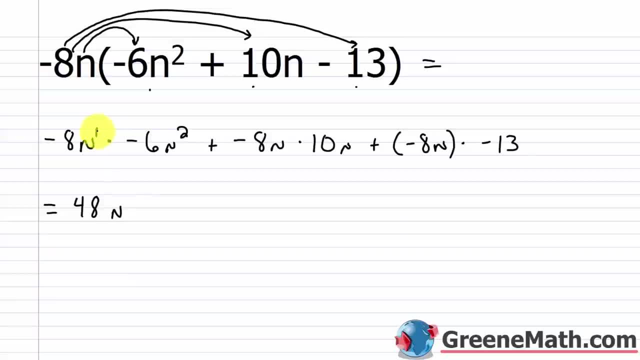 And then we just add the exponents. Remember this has an exponent of one. So one plus two would give me three. So this is 48 n cubed. Then next I have it: Negative eight n times 10 n. 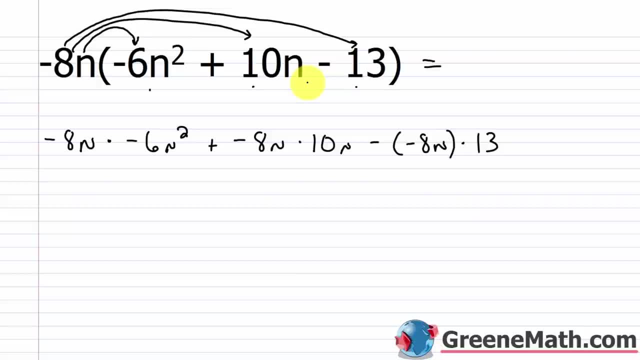 And one of the things you can do here, you can think about this as negative 13. Right? So you don't make a sign mistake. Or you can have a minus. You'd end up with minus and negative. 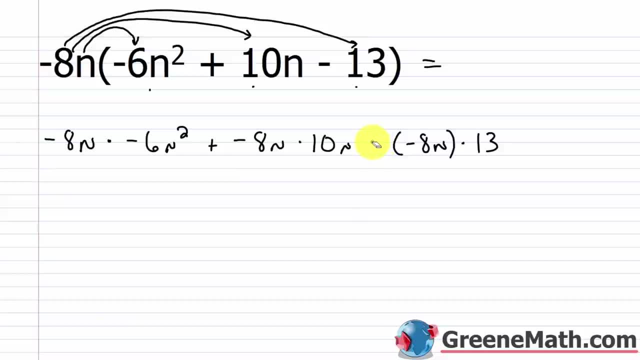 We know that would be plus a positive. But just to make this easy on us, I'm just going to put plus right here. And I'm going to write this as a negative 13. Okay. 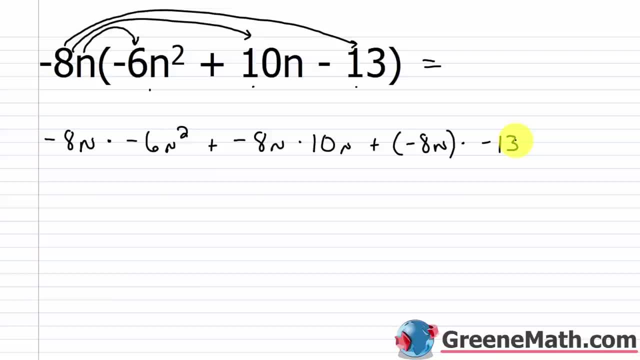 So let's go through and crank out the multiplication. So negative 8n times negative 6n squared. Negative 8 times negative 6 is, first off, a positive. Right? 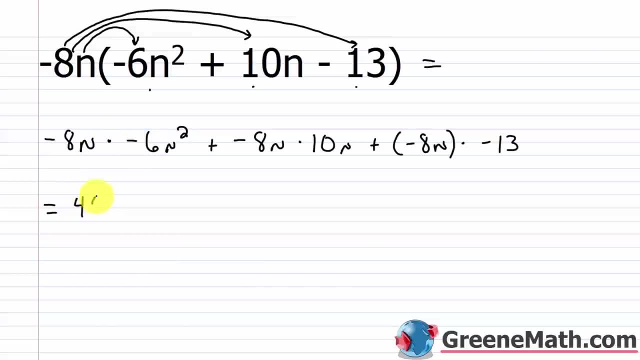 Negative times negative is positive. 8 times 6 is 48. And then if we have n times n squared. Well, the base n stays the same. And then we just add the exponents. Remember, this has an exponent of 1. So 1 plus 2 would give me 3. So this is 48n cubed. 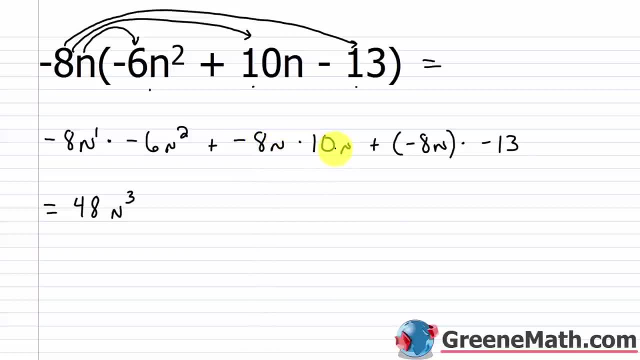 Then next I have negative 8n times 10n. Well, negative 8 times 10 is negative 80. So minus 80. 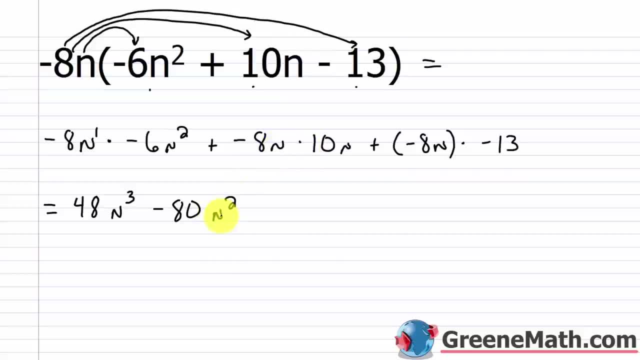 And then n times n is n squared. Again, keep the base n the same. And you add your exponents. Right? Each case has an exponent of 1. 1 plus 1 is 2. So you get n squared. 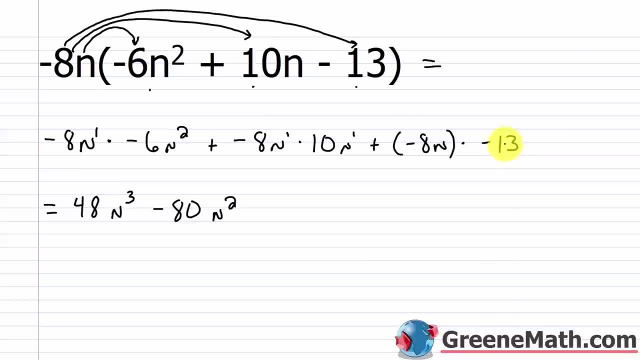 Then we have negative 8n times negative 13. So negative times negative is positive. And 8 times 13 is 104. So this would be 104. And then don't forget the n. So there's your answer. You get 48n cubed minus 80n squared plus 104n. 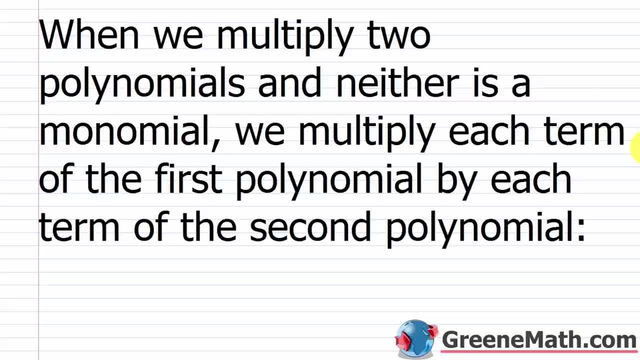 All right. So now that we've seen how to multiply a monomial, which, again, is a polynomial with one single term, times a polynomial. And the specific examples we looked at, we looked at multiplying by a binomial, which is a polynomial with two terms, and a trinomial, which is a polynomial with three terms. 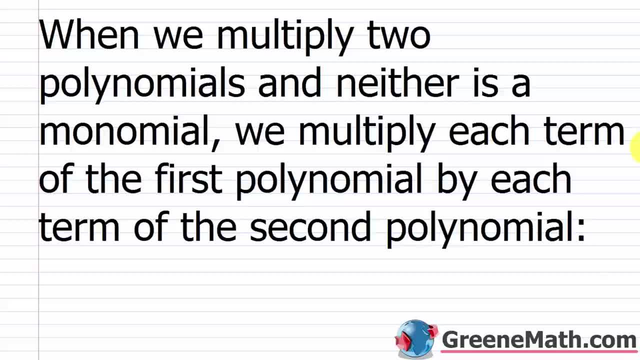 But that really doesn't matter because if I had a polynomial with four terms or five terms or whatever, it would be the same process. 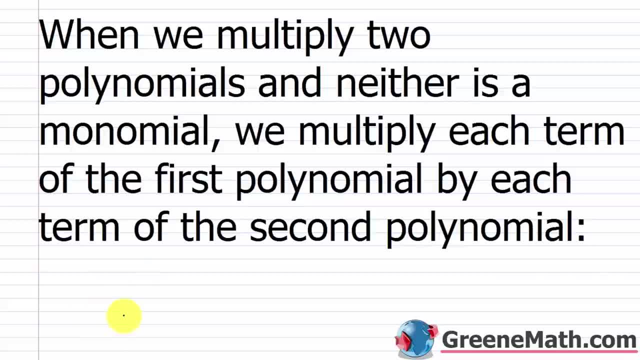 I would take the monomial and I would multiply it by each term in that polynomial. Okay. That's all we need to do. We're using our distributive property. 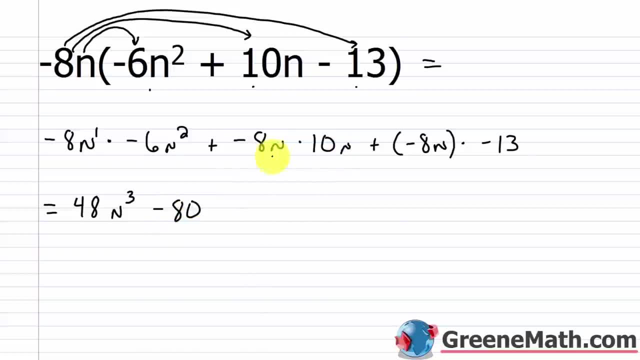 Well, negative eight times 10 is negative 80,, so minus 80. And then n times n is n squared Again. keep the base n the same and you add your exponents right. Each case has an exponent of one. 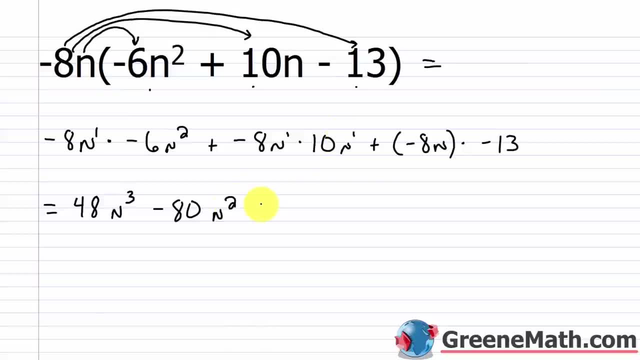 One plus one is two, so you get n squared. Okay, then we have negative eight n times negative, 13. So negative times negative is positive, And eight times 13 is 104. So this would be 104.. And then, don't forget, negative eight n times 10, n squared. 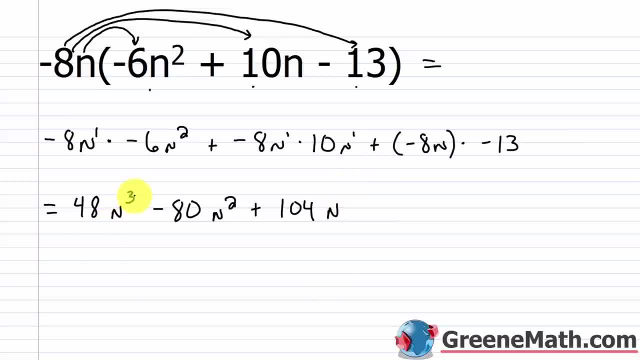 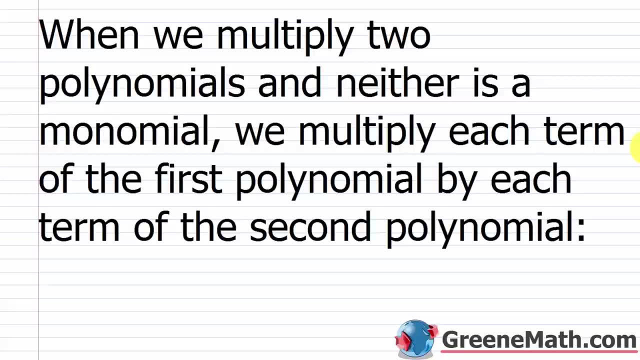 Don't forget the n. So there's your answer: You get 48 n cubed minus 80 n squared, plus 104 n. All right. so now that we've seen how to multiply a monomial, which again is a polynomial, with, 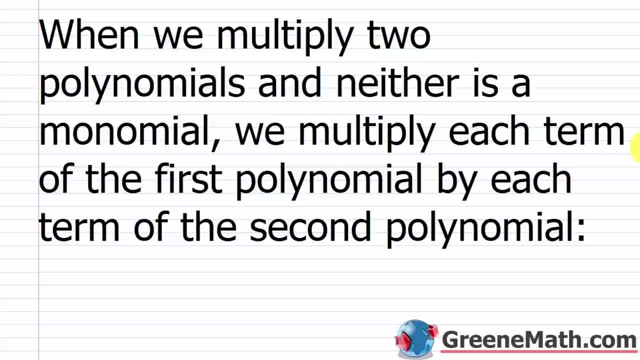 one single term times a polynomial and the specific examples we looked at. we looked at multiplying by a binomial, which is a polynomial with two terms, and a trinomial, which is a polynomial with three terms. But that really doesn't matter, because if I had a polynomial with four terms or five, 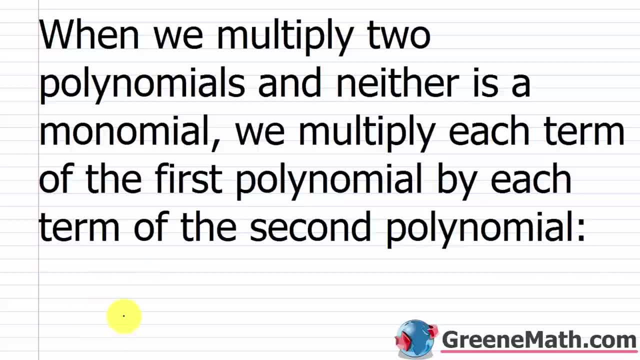 terms or whatever. It's the same process. I would take the monomial and I would multiply it by each term in that polynomial. okay, That's all we need to do. We're using our distributive property. Now we multiply two polynomials and neither is a monomial, okay. 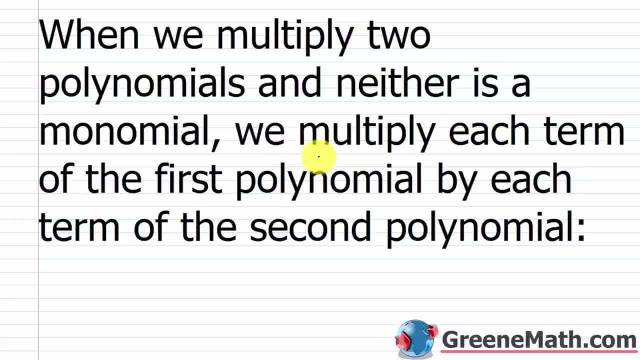 Neither one is a monomial. We multiply each term of the first polynomial, each term of the first polynomial, by each term of the second polynomial. So let me show you that. Let's say we have something like negative four x minus four. 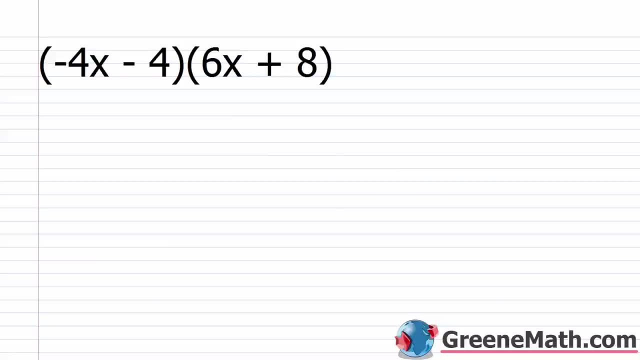 And we're multiplying this by six x plus eight. So this is the product of two binomials, And this is going to happen so often. we have like a little shortcut for this, called FOIL, And I'm going to teach you that in the next lesson. 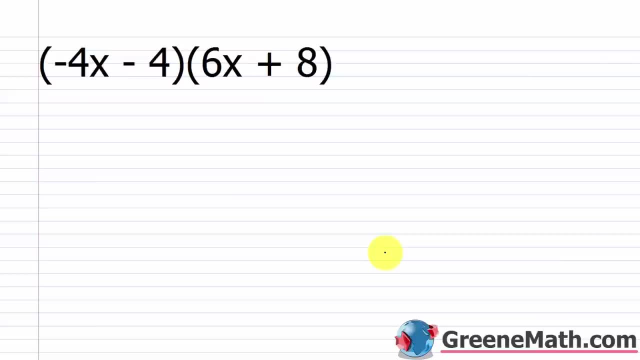 But for right now I'm going to kind of show you a general method to do this. So I'm just going to take each term of the first polynomial and multiply it by each term of the second polynomial. So I'm going to break this up into two different problems. 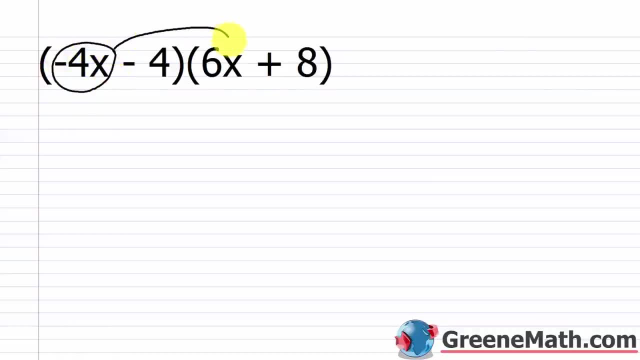 So I'm going to have negative four x, Multiply, Multiply, Multiply, Multiply, Multiply. So I'll have negative four x multiplied by six x plus eight, And then I'm going to add to that, I'm going to take negative four and I'm going to multiply. Now we multiply two polynomials and neither is a monomial. Okay. Neither one is a monomial. 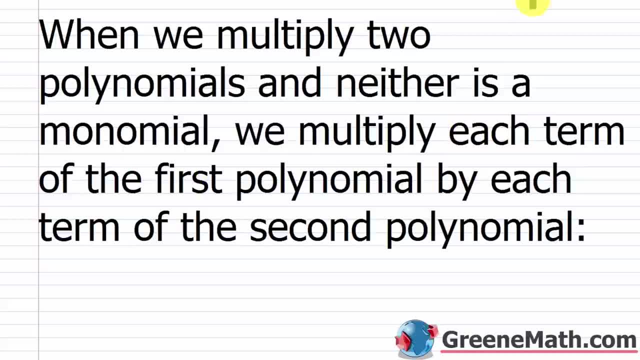 We multiply each term of the first polynomial. Each term of the first polynomial 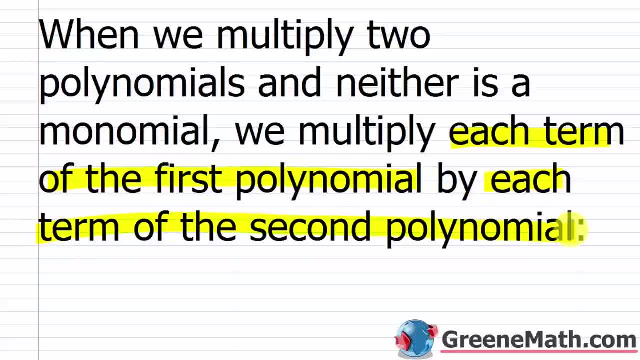 by each term of the second polynomial. 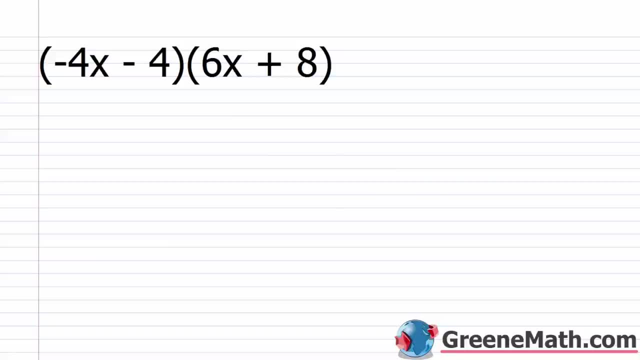 So let me show you that. Let's say we have something like negative 4x minus 4 and we're multiplying this by 6x plus 8. 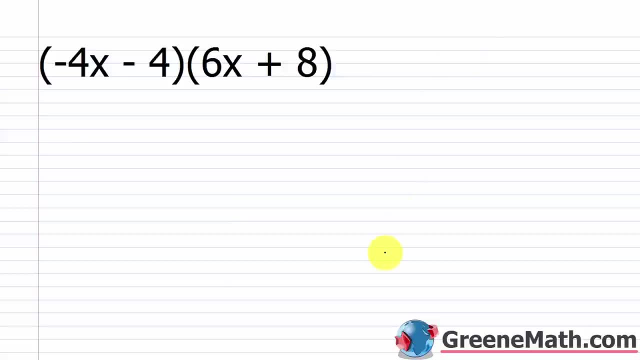 So this is the product of two binomials. And this is going to happen so often, we have like a little shortcut for this called FOIL. And I'm going to teach you that in the next lesson. 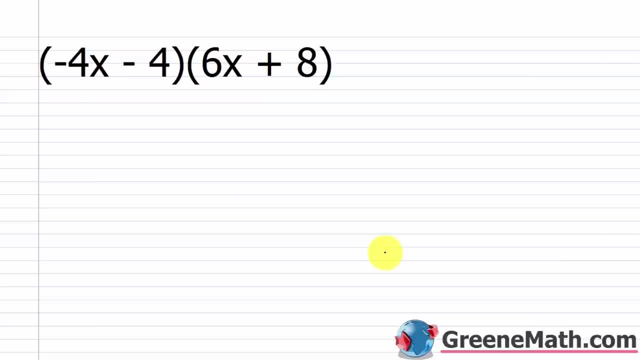 But right now I'm going to kind of show you a general method to do this. 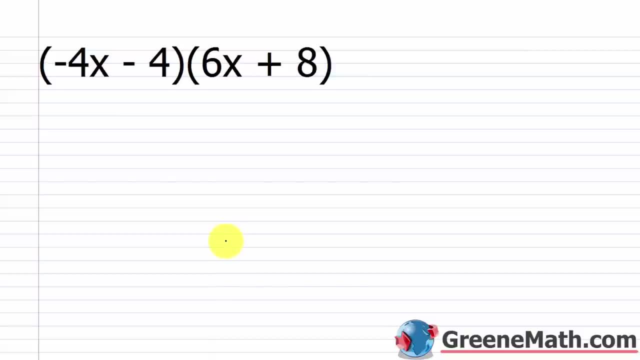 So I'm just going to take each term of the first polynomial and multiply it by each term of the second polynomial. So I'm going to break this up into two different problems. 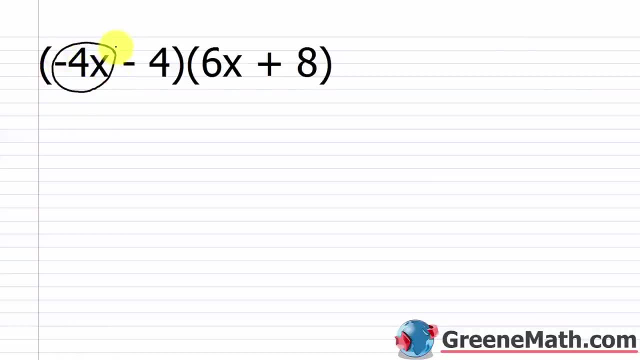 So I'm going to have negative 4x multiplied by this 6x plus 8. So I'll have negative 4x multiplied by 6x plus 8. And then I'm going to add to that, I'm going to take negative 4 and I'm going to multiply it again by 6x plus 8. 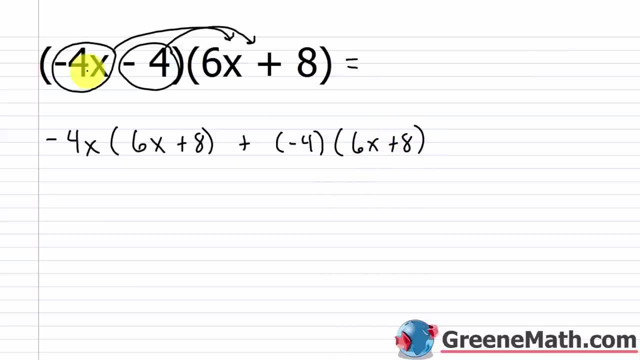 So this is each term of the first polynomial being multiplied by each term of the second polynomial. 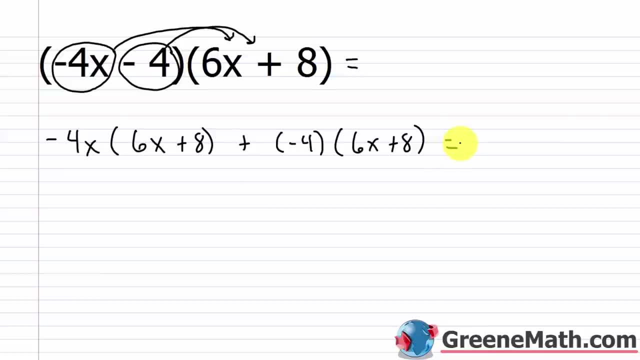 So again, now I'm just going to use my distributive property, just like I used in the previous example. 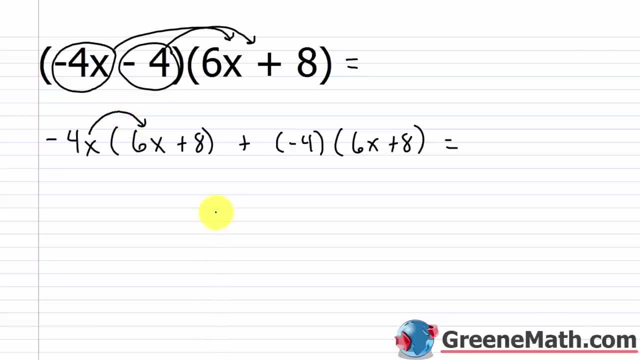 So for the first one, I would do negative 4x times 6x. So I'd have negative 4 times 6, that's negative 24. 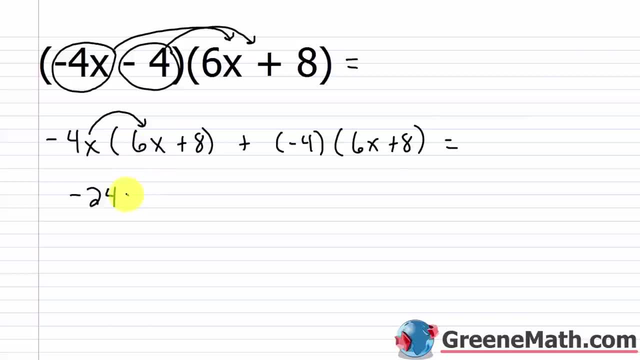 And then x times x is x squared. 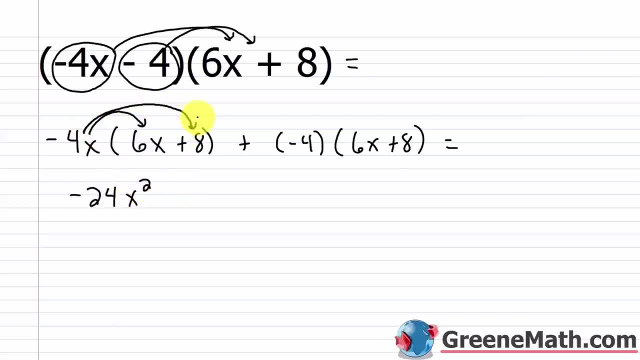 Then I'd have negative 4x times 8. So I know negative times positive is negative, so I'm going to put a minus there. 4 times 8 is 32. 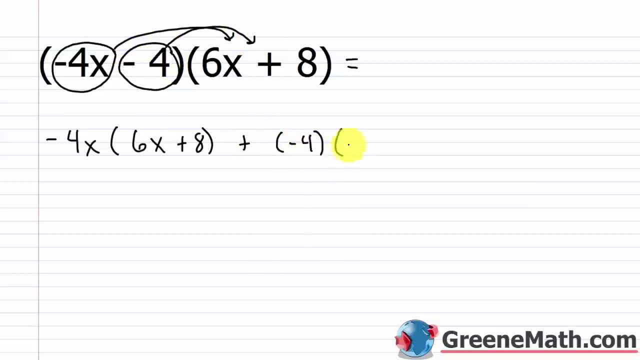 it again by six x plus eight. So this is each term of the first polynomial being multiplied by each term of the second polynomial. So again now I'm just going to use my distributive property, just like I used in the previous example. 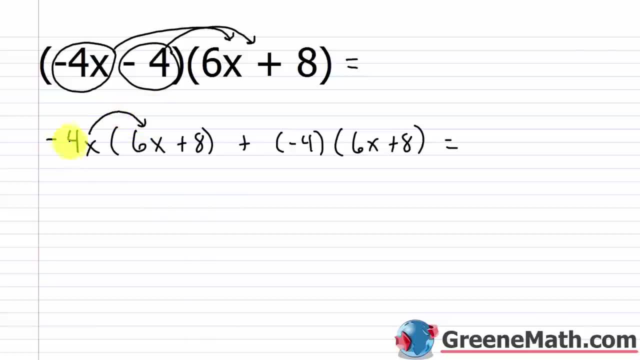 Okay, Okay, Okay. do negative 4x times 6x. So I'd have negative 4 times 6, that's negative 24. and then x times x is x squared. Then I'd have negative 4x times 8.. So I know negative times positive is negative. so I'm. 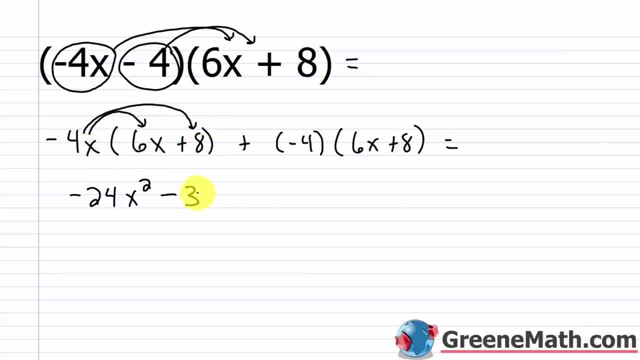 going to put a minus there. 4 times 8 is 32, and then x will come along for the ride. So the result from this is negative 24x squared minus 32x. All right now. next we're looking over here. I have 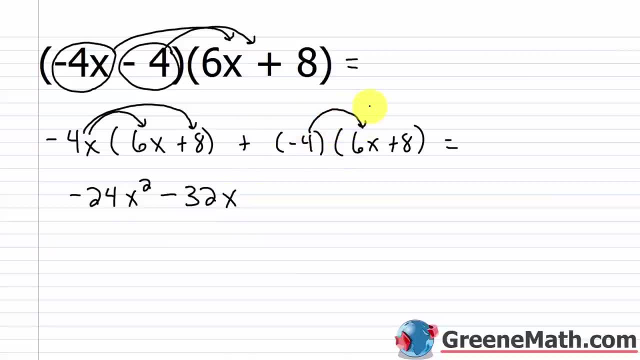 plus and then negative 4 times 6x. So negative times positive is negative 4 times 6 is 24.. So I'd have 24, and then x comes along for the ride, So minus 24x, and then I have negative 4 times 8.. 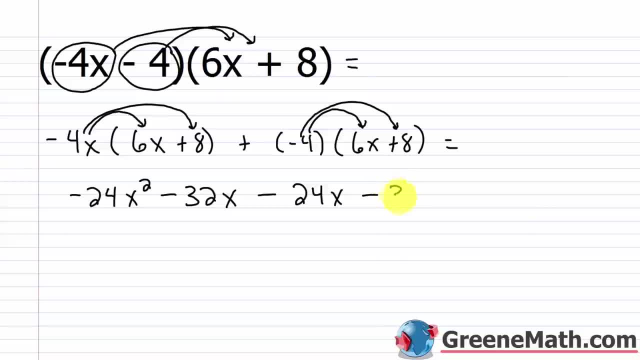 So negative times positive is negative. 4 times 8 is 32.. So I'm not done. In the previous exam I never had any like terms or anything. I would not report this as my answer, because I have negative 32x and I have negative 24x. Those can be combined right. They're like terms. So what is? 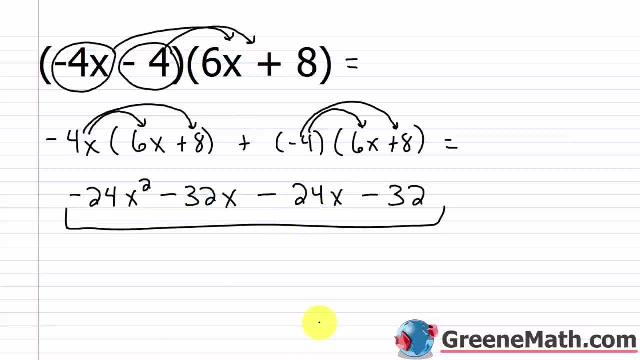 negative 32 minus 24?? Well, that's negative 56.. So this is going to end up being negative 24x squared minus 56x minus 32.. That would be my answer. All right, let's take a look at another one. 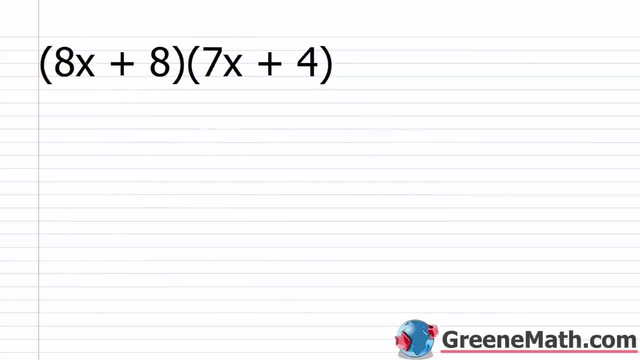 We have 8x plus 8 times 7x squared. So again, I'm going to take each term of the first polynomial and multiply it by each term of the second polynomial. So I'm going to do 8x times 7x plus 4.. So 8x times 7x plus 4.. And then plus. 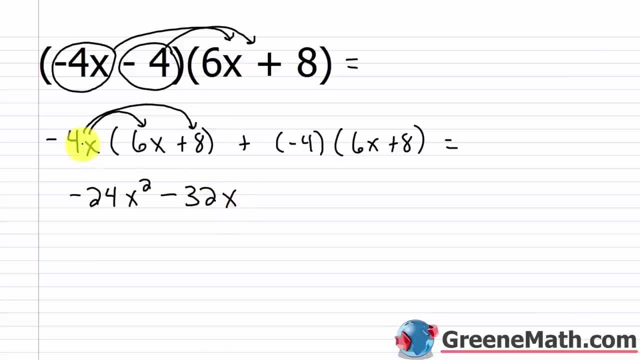 And then x will come along for the ride. So the result from this is negative 24x squared minus 32x. 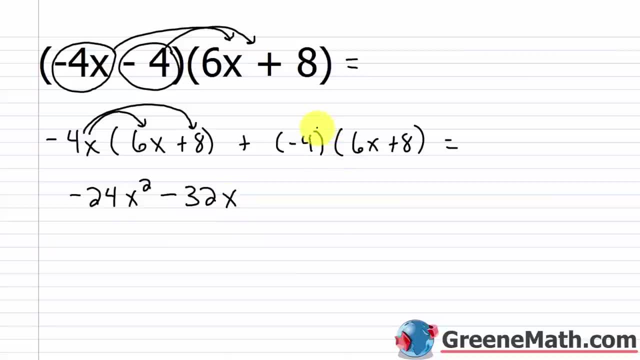 Alright, now next we're looking over here. I have plus and then negative 4 times 6x. 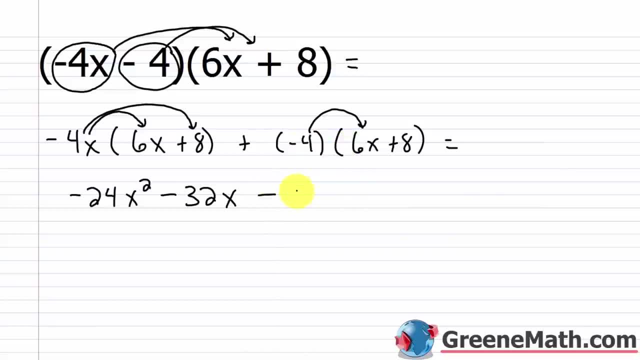 So negative times positive is negative. 4 times 6 is 24. So I'd have 24 and then x comes along for the ride. 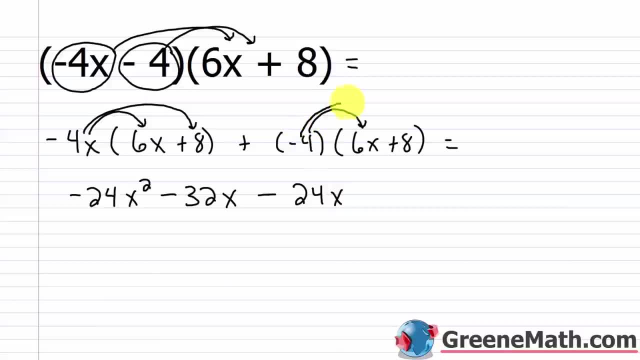 So minus 24x. And then I have negative 4 times 8. 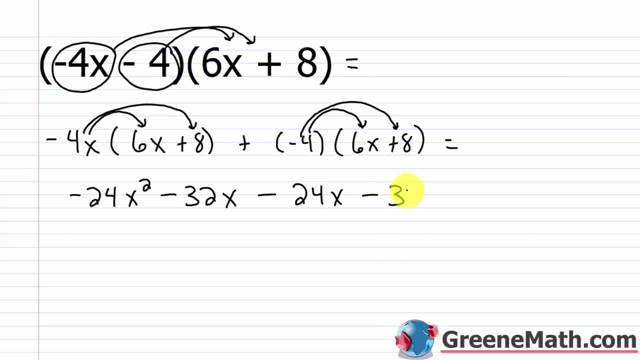 So negative times positive is negative. 4 times 8 is 32. So I'm not done. 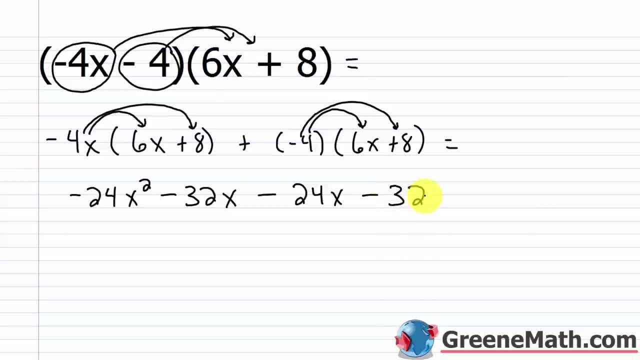 In the previous examples, I never had any like terms or anything. I would not report this as my answer because I have negative 32x and I have negative 24x. 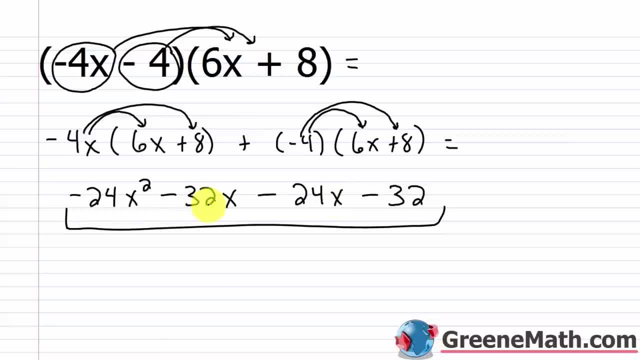 Those can be combined, right? They're like terms. So what is negative 32 minus 24? Well that's negative 56. 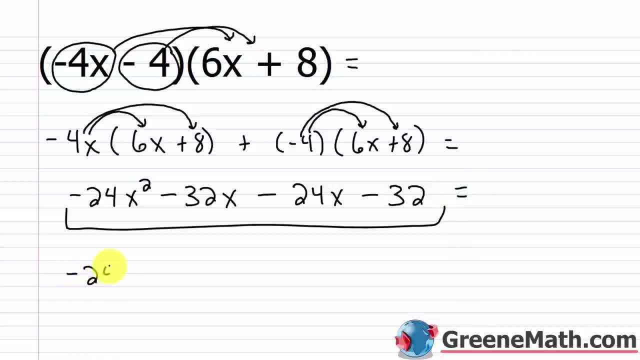 So this is going to end up being negative 24x squared minus 56x minus 32. That would be my answer. 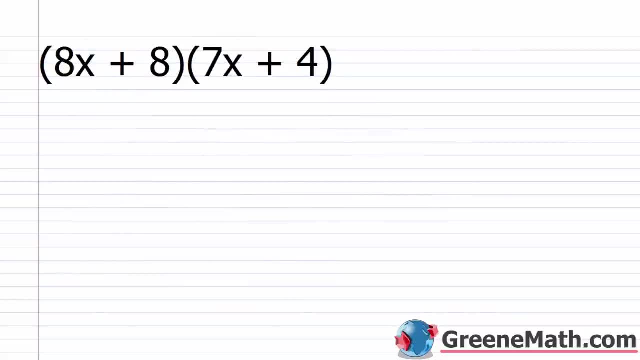 Alright, let's take a look at another one. We have 8x plus 8 times 7x plus 4. So again, I'm going to take each term of the first polynomial and multiply it by each term of the second polynomial. 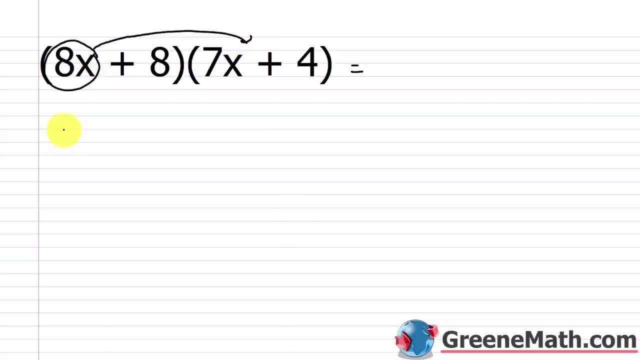 So I'm going to do 8x times 7x plus 4. So 8x times 7x plus 4. And then plus, next I'm going to do 8 times, again, 7x plus 4. 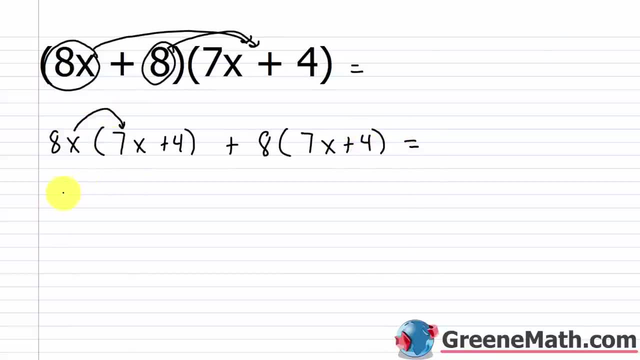 Alright, so I'm going to do 8x times 7x. 8 times 7 is 56. x times x is x squared. Then next I'd have 8x times 4. 8 times 4 is 32. 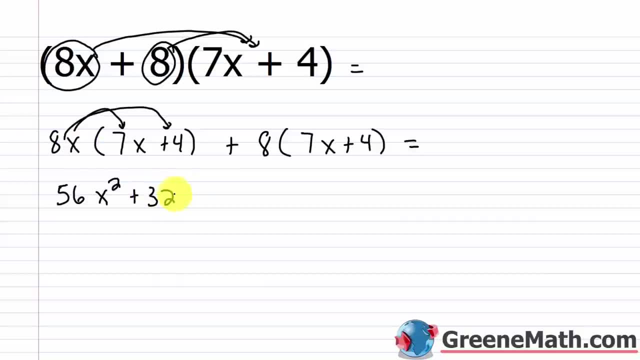 So I'm going to put plus 32. And then x comes along for the ride. 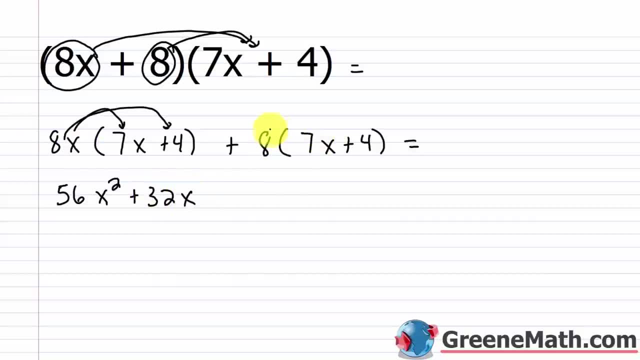 So plus 32x. Alright, then next I have 8 times 7x. 8 times 7 is 56. And then x would come along for the ride. So this is plus 52x. And lastly I have 8 times 4. 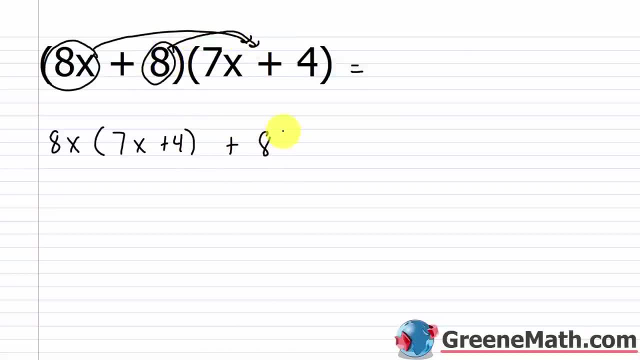 Next I'm going to do 8 times again, 7x plus 4.. All right, so I'm going to do 8x times 7x. 8 times 7 is 56.. x times x is x squared. The next I'd have 8x times 4.. 8 times 4 is 32.. So I'm going to put plus 32.. And then x comes along. 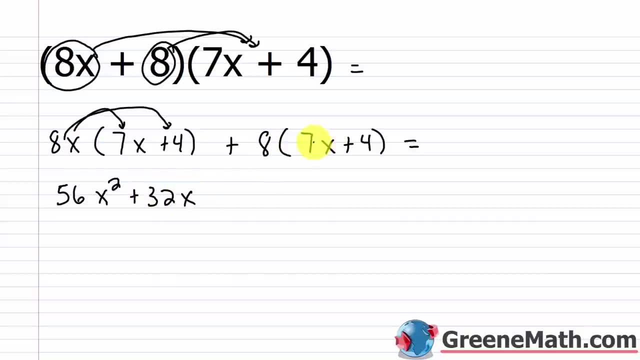 for the ride. So plus 32x. All right, the next I have 8 times 7x. 8 times 7 is 56., And then x would come along for the ride. So this is plus 56x. And lastly, I have 8 times 4. And that's 32.. So plus 32.. 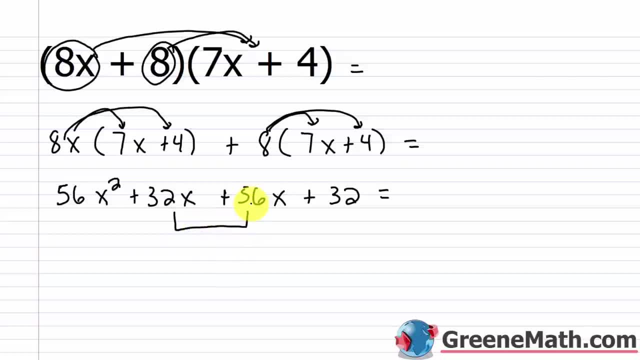 And again I have like terms that I can combine here. So I have to do 56x squared Plus 32x plus 56x is 88x And then plus 32.. So that's my answer: 56x squared plus 88x plus 32.. 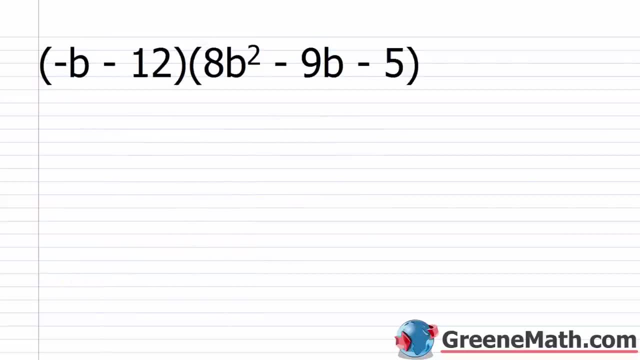 All right, for the next one, I have a binomial multiplied by a trinomial, So nothing's going to change here. I'm still going to multiply each term of the first polynomial by each term of the second polynomial. So I have negative b minus 12 times 8b squared minus 9b minus 12.. So that's. 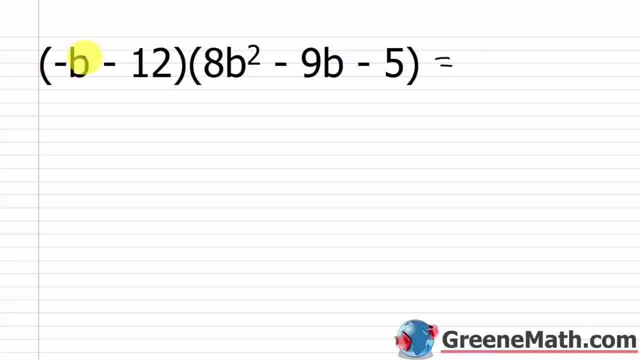 minus 5.. All I'm going to do is I'm going to take this guy right here, negative b And I'm going to multiply it by this whole thing here. So negative b times inside of parentheses: 8b squared minus 9b. 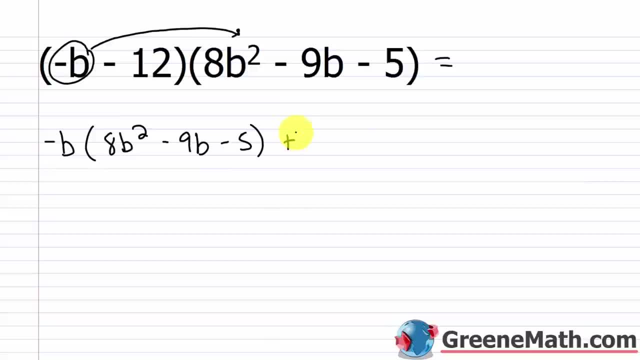 minus 5.. And then I'm going to put plus. Next I have this negative 12.. Okay, negative 12 times this whole quantity, Negative 12 outside of the parentheses, And then inside of parentheses we'll have 8b squared minus 9b. 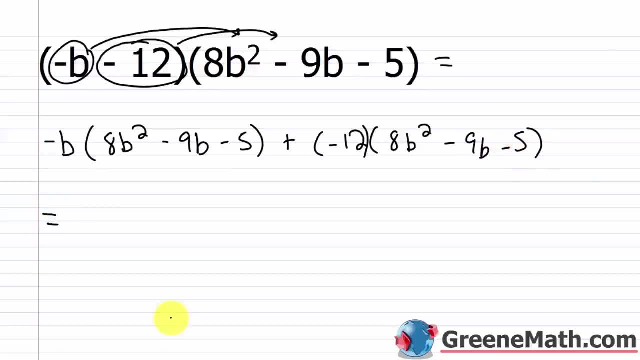 Minus 5.. Let's go ahead and crank this out. So I'll have negative b times 8b squared, Negative times positive is negative, And then you basically have b times b squared. That's b cubed, So you would have 8.. That comes along for the ride And then b cubed, All right. so negative, 8b cubed, And 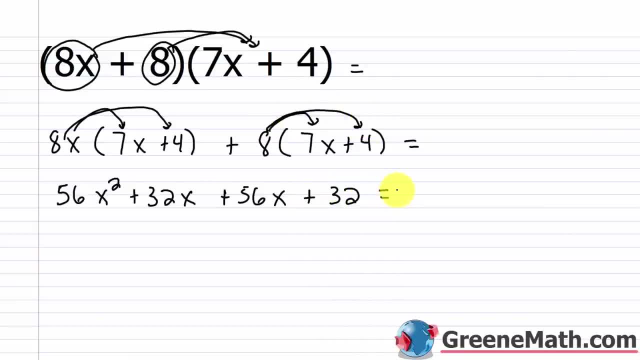 And that's 32. So plus 32. And again, I have like terms that I can combine here. So I have to do 56x squared plus 32x plus 56x is 88x. And then plus 32. So that's my answer. 56x squared plus 88x plus 32. 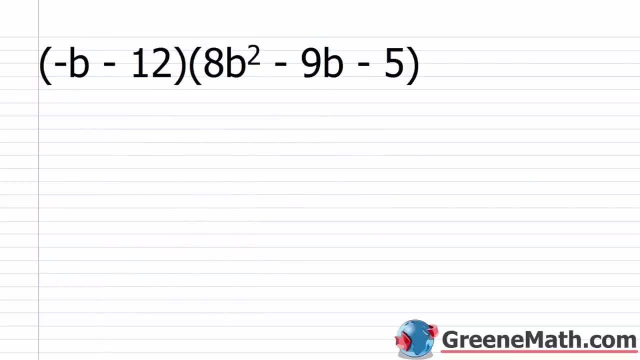 Alright, for the next one I have a binomial multiplied by a trinomial. So nothing's going to change here. I'm still going to multiply each term of the first polynomial by each term of the second polynomial. So I have negative b minus 12 times 8b squared minus 9b minus 5. All I'm going to do is I'm going to take this guy right here, negative b. And I'm going to multiply it by this whole thing here. So negative b times inside of parentheses 8b squared minus 9b minus 5. And then I'm going to put plus. 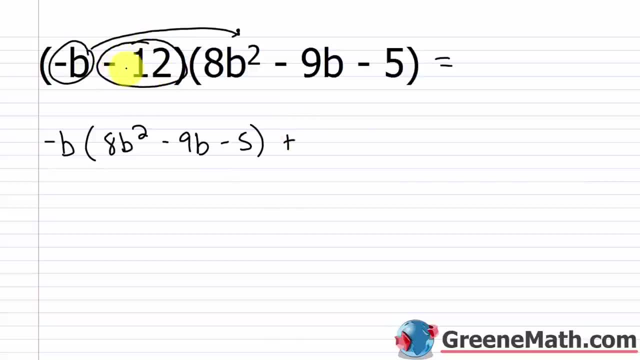 Next I have this negative 12. Okay, negative 12 times this whole quantity. Negative 12 outside of the parentheses and then inside of parentheses. We'll have 8b squared minus 9b minus 5. 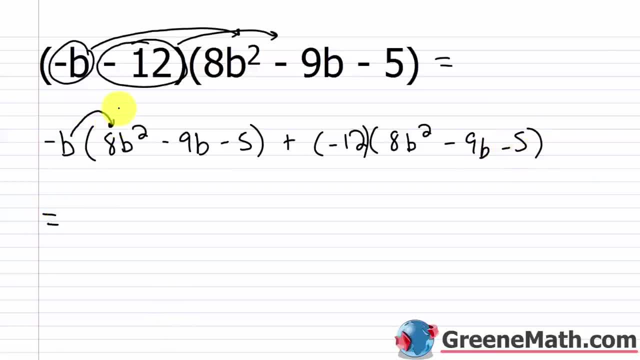 Let's go ahead and crank this out. So I'll have negative b times 8b squared. Negative times positive is negative. And then you basically have b times b squared. That's b cubed. So you would have 8. That comes along for the ride. 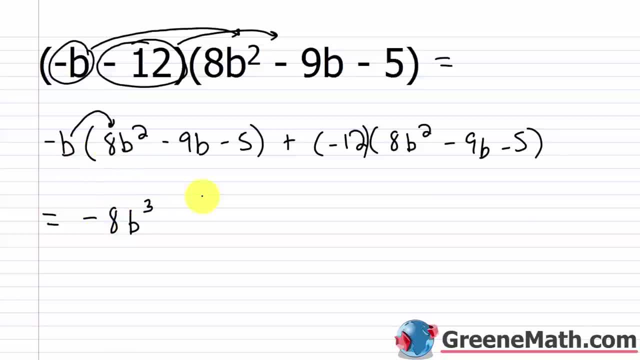 And then b cubed. All right, so negative 8b cubed. 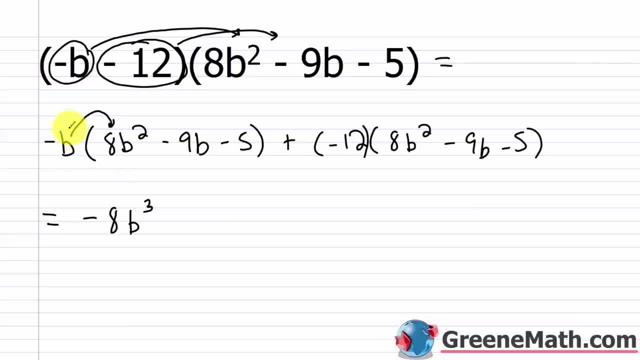 And then the next one, we'd have a negative b times a negative 9b. So negative times negative is positive. b times b is b squared. 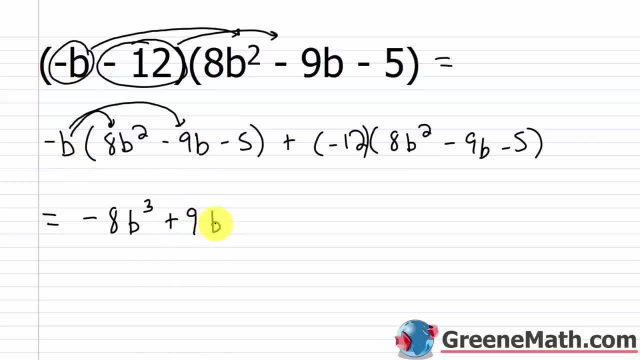 So this would be positive 9b squared. Then I'd have negative b times negative 5. 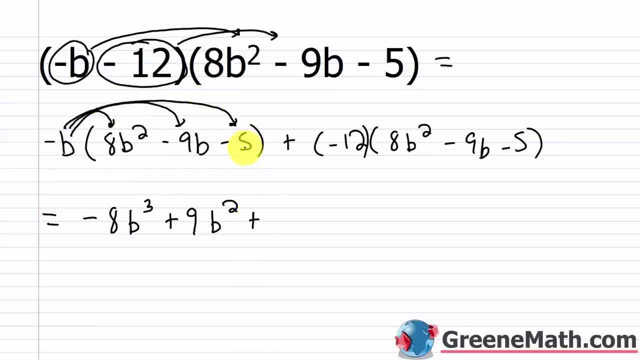 So negative times negative is positive. You have b times 5. That's just 5b. 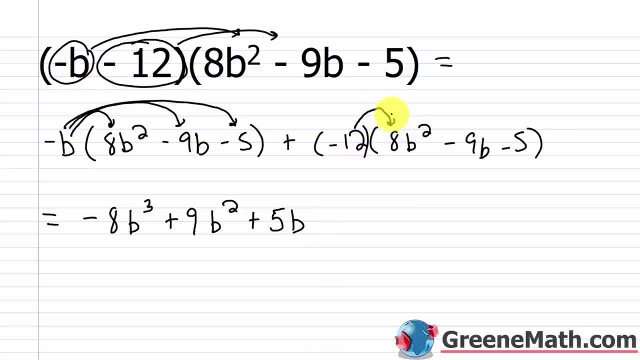 Now I'm moving on to this over here. I'll have negative 12 times 8b squared. 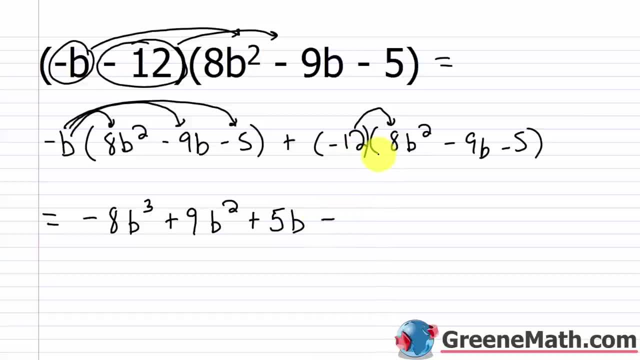 Negative times positive is negative. 12 times 8 is 96. So this would be minus 96b squared. 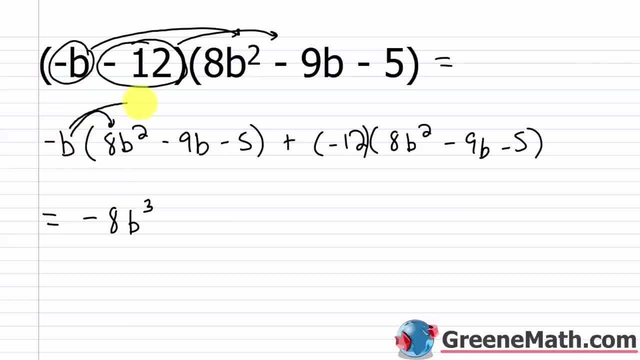 then the next one. we'd have a negative b times a negative 9b. So negative times negative is positive. b times b is b squared, So this will be positive, And then negative times negative is positive 9b squared. Then I'd have negative b times negative, 5.. So negative times negative is. 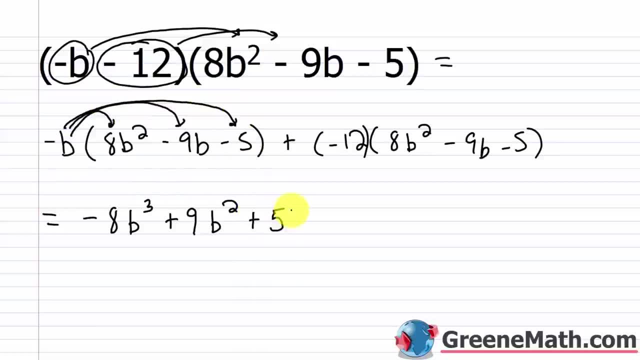 positive, You have b times 5.. That's just 5b. Okay, now, moving on to this, over here I'll have negative 12 times 8b squared. Negative times positive is negative. 12 times 8 is 96.. So this: 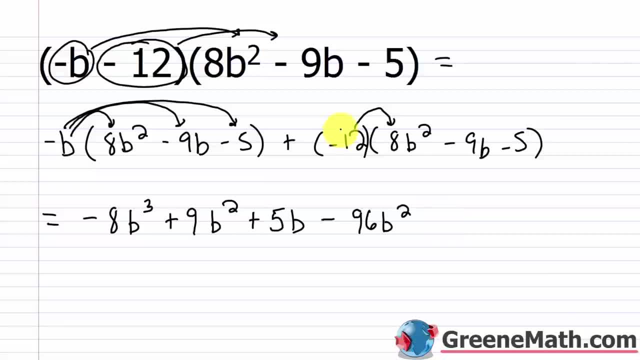 would be minus 96b squared. Then next I have negative- 12 times negative- 9b. Negative times negative is positive. 12 times 9 is 108. So this would be 108b. Then, lastly, I have negative 12. 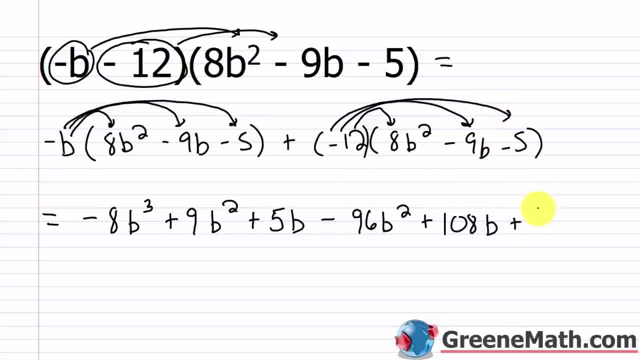 times negative: 5.. Negative times negative is positive. 12 times 5 is 60. So we have negative 8b cubed plus 9b squared plus 5b, minus 96b, squared plus 108b plus 60. So where are my like terms here? 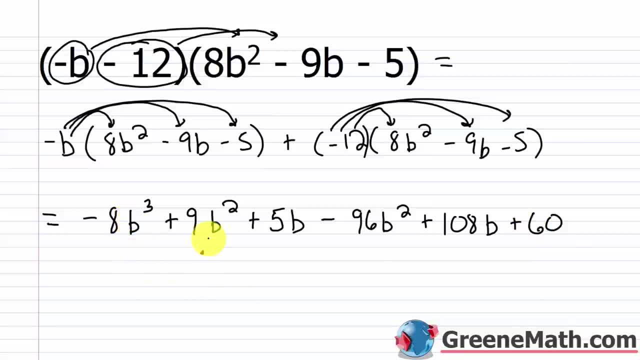 Nothing to combine with this one. But I have 9b squared and I have negative 96b squared. Those are like terms. And then I have 5b and I have 108b. Those are like terms. So we want to simplify by combining like terms here before we report our. 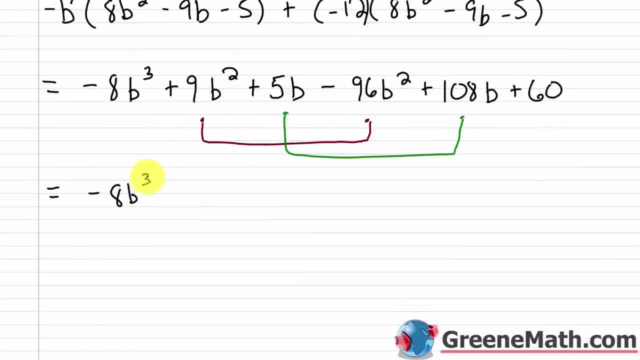 answer. So negative 8b cubed, That's going to stay the same. And then 9b squared minus 96b squared, That's going to be negative 87b squared. And then I have 5b plus 108b, That's going to be plus 113b, And then finally plus 60.. So there's your answer. 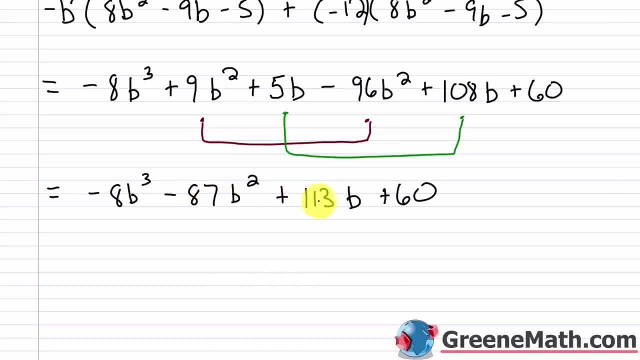 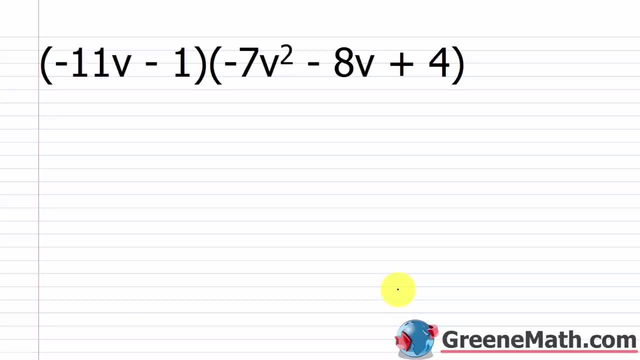 Negative 8b cubed minus 87b squared plus 113b plus 60.. All right, for the next one, I have negative 11v minus 1. And we're multiplying this by negative 7v squared minus 8v plus 4.. So again I'm going. 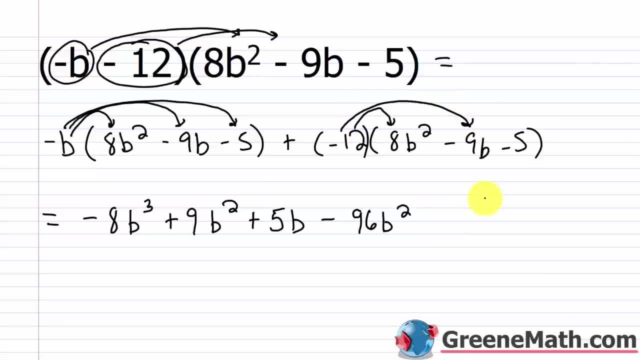 Then next I have negative 12 times negative 9b. Negative times negative is positive. 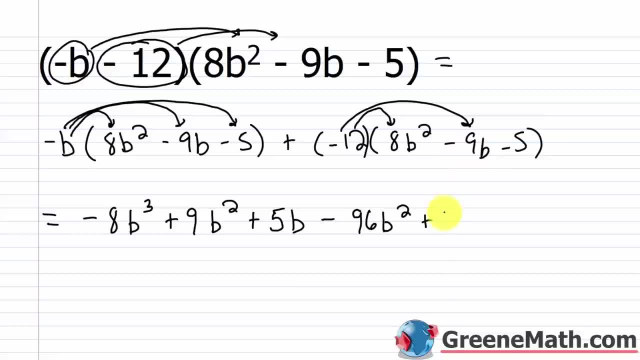 12 times 9 is 108. So this would be 108b. 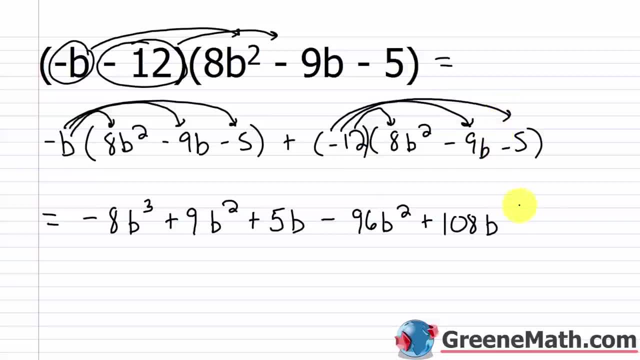 Then lastly, I have negative 12 times negative 5. Negative times negative is positive. 12 times 5 is 60. 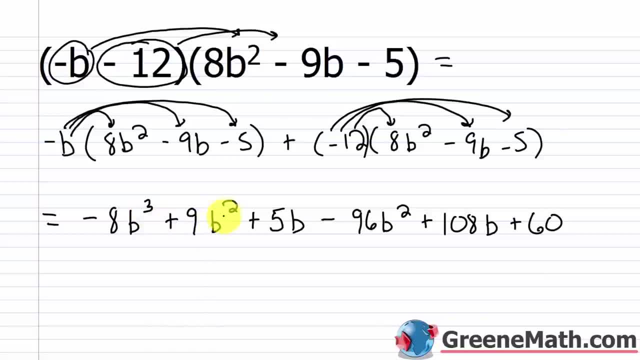 So we have negative 8b cubed plus 9b squared plus 5b minus 96b squared plus 108b plus 60. 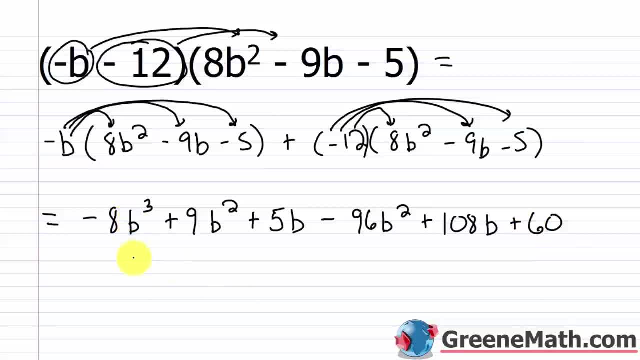 So where are my like terms here? Nothing to combine with this one. 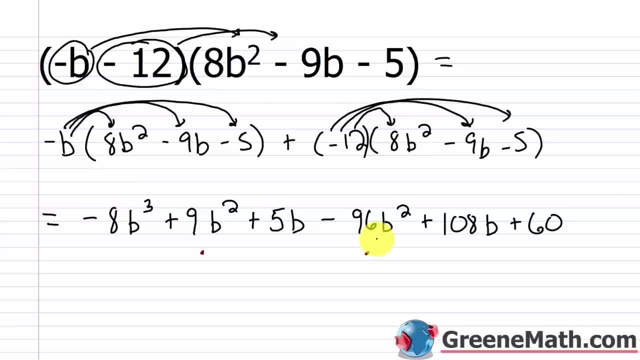 But I have 9b squared and I have negative 96b squared. Those are like terms. And then I have 5b and I have 108b. Those are like terms. 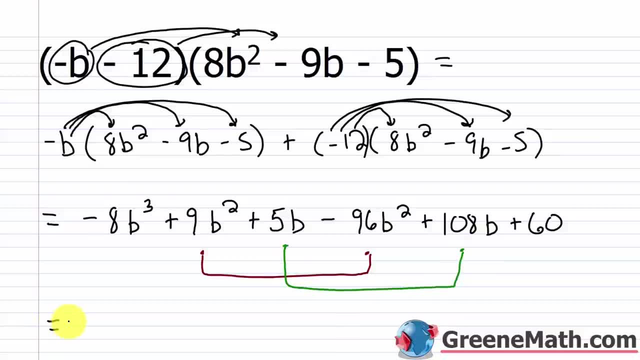 So we want to simplify by combining like terms here before we report our answer. 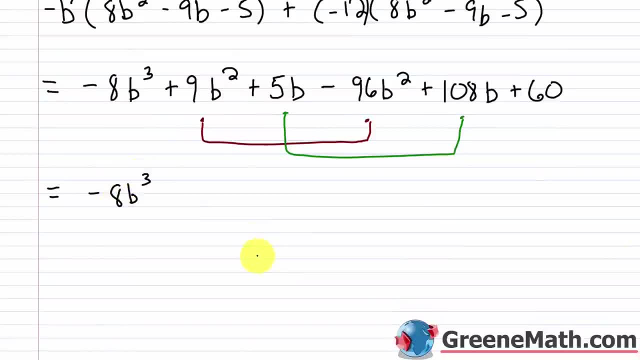 So negative 8b cubed, that's going to stay the same. And then 9b squared minus 96b squared. That's going to be negative 87b squared. And then I have 5b plus 108b. 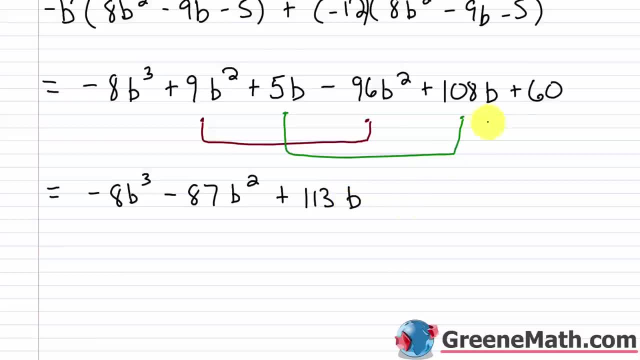 That's going to be plus 113b. And then finally plus 60. So there's your answer. 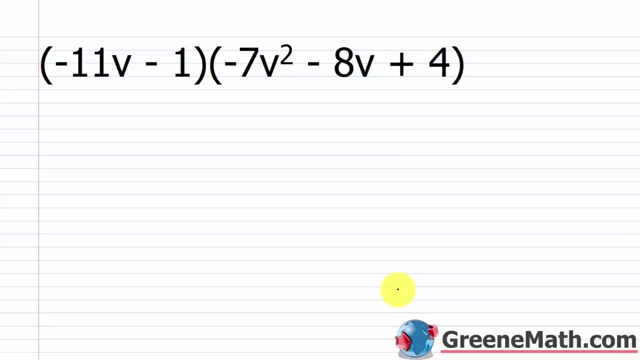 Alright, for the next one I have negative 11v minus 1. And we're multiplying this by negative 7v squared minus 8v plus 4. So again, I'm going to take each term of the first polynomial and multiply it by each and every term of the second polynomial. So I'm going to take this negative 11v, multiply it by this guy. So negative 11v times, you have negative 7v squared minus 8v. 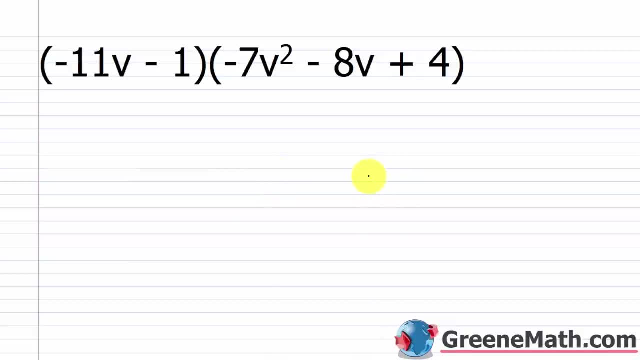 to take each term of the first polynomial and multiply by each and every term of the second polynomial. So I'm going to take this and I'm going to multiply by each and every term of the second polynomial. So I'm going to take this negative 11v multiplied by this guy. So negative 11v times you have negative. 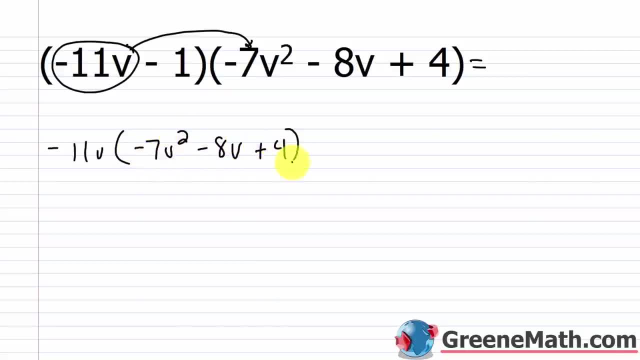 7v squared minus 8v plus 4.. And then plus. Next I'm going to take negative 1 and multiply it by this guy as well. So plus negative 1 times negative 7v squared minus 8v plus 4.. So negative 11v times. 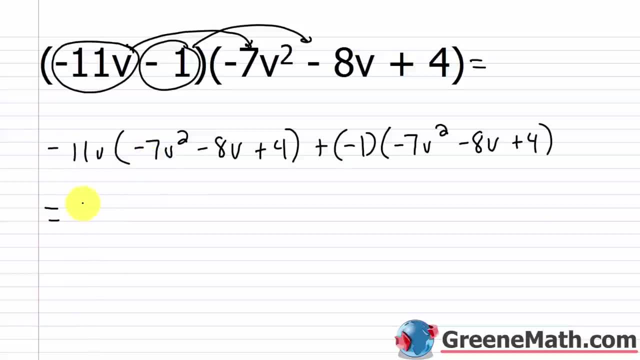 negative: 7v squared Negative 11 times negative: 7. Is 77.. V times v squared is v cubed Negative 11v times negative. 8v. Negative times negative is positive 11 times 8 is 88.. V times v is v squared Negative 11v times 4 would be negative And then 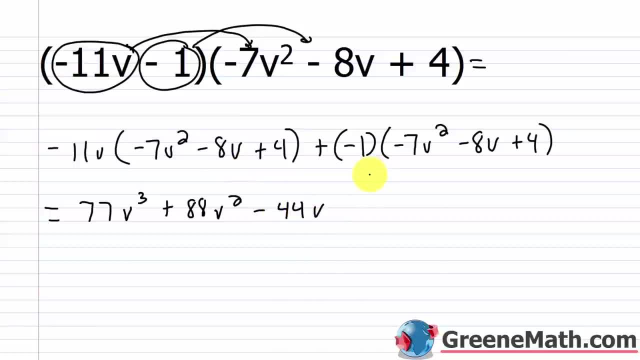 11 times 4 is 44.. And then v. All right, then, moving on over here, I have negative 1 times negative 7v squared. It's basically just a sign. change right, You multiply by negative 1, you're just changing. 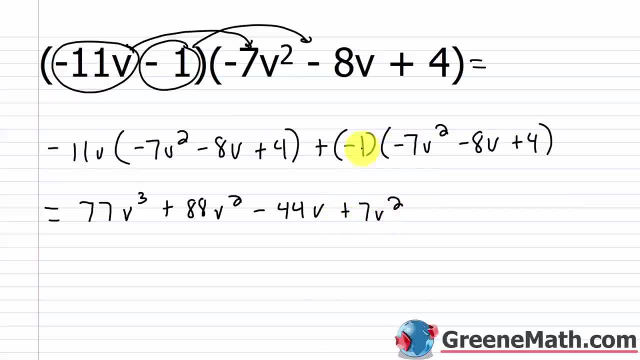 the sign. So this would be negative 1 times negative 7v squared. So negative 1 times negative 7v squared. Negative 1 times negative 8v. That would be plus 8v Again, just changing the sign. 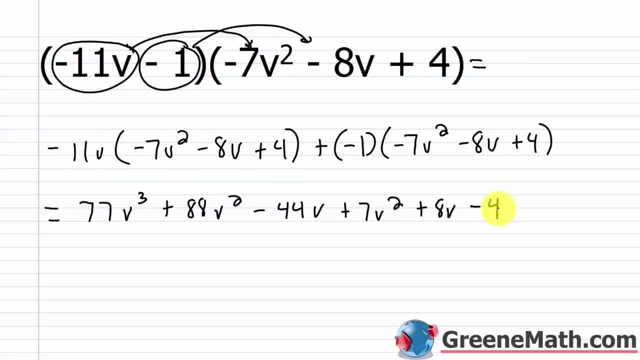 Negative 1 times 4 would be minus 4.. Again, lastly, just changing the sign. All right, so now let's look for a like term. So 77v cubed. Nothing I can combine with that 88v squared and 7v squared. 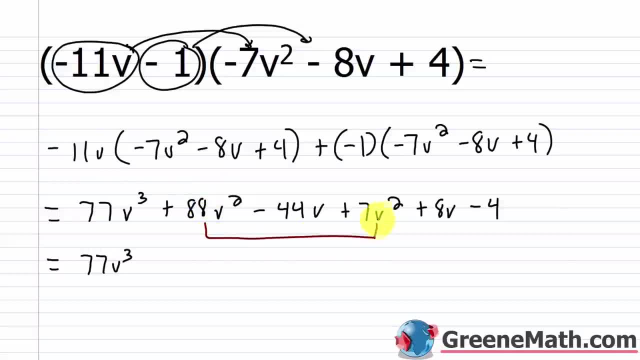 Those are like terms. These are like terms. So what is 88 plus 7?? Well, that's 95.. So then plus 95v squared, And then for other like terms, we have negative 44v and 8v. Those are like terms. 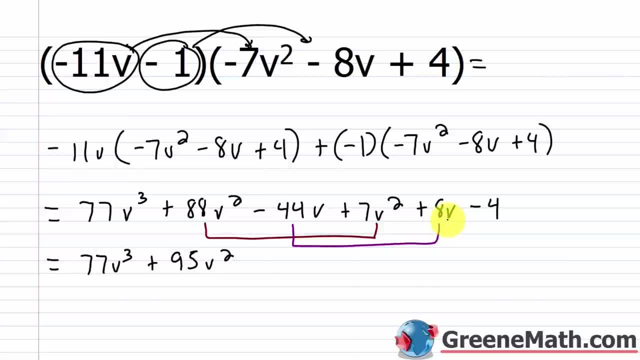 So if we can combine those, you'd end up with negative 36v, So minus 36v, And then, lastly, minus 4.. So we end up with 77v cubed plus 95v squared, minus 36v minus 4.. All right, let's take 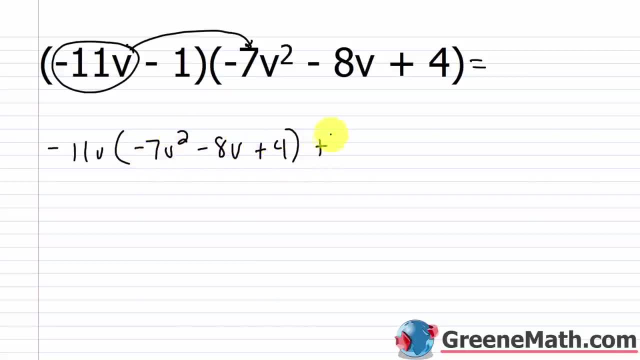 Plus 4. And then plus, next I'm going to take negative 1 and multiply it by this guy as well. So plus negative 1 times negative 7v squared minus 8v plus 4. So negative 11v times negative 7v squared. Negative 11 times negative 7 is 77. V times v squared is v cubed. Negative 11v times negative 8v. Negative times negative is positive. 11 times 8 is 88. V times v is v squared. 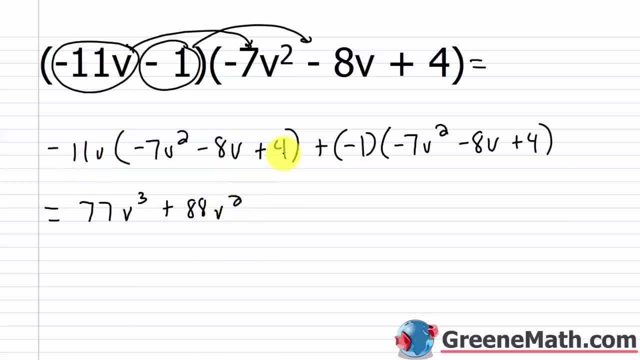 Negative 11v times 4 would be negative. And then 11 times 4 is 44. And then v. Alright, then moving on over here. 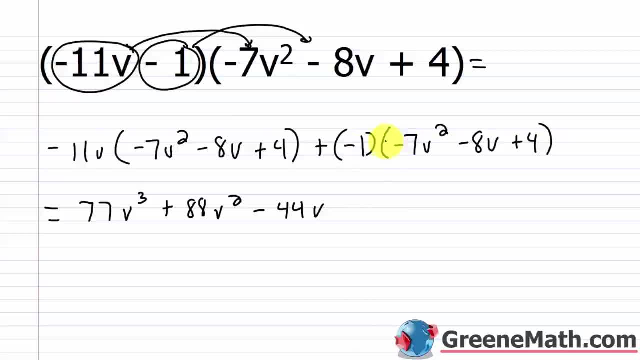 I have negative 1 times negative 7v squared. It's basically just a sign change, right? You multiply by negative 1, you're just changing the sign. So this would be plus 7v squared. 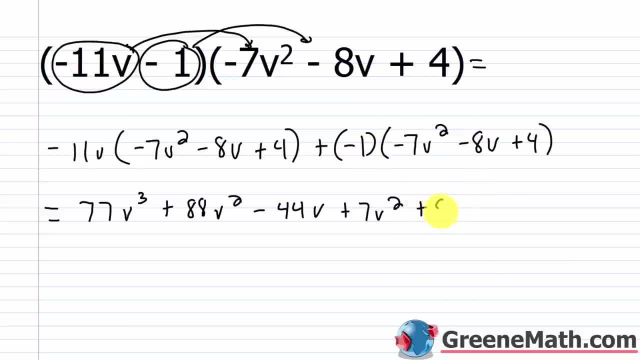 Negative 1 times negative 8v. That would be plus 8v. Again, just changing the sign. Negative 1 times 4 would be minus 7v squared. 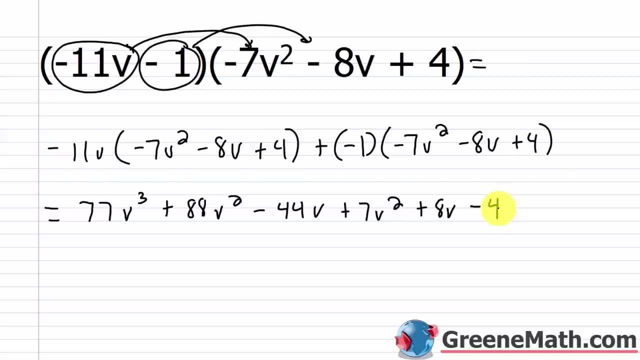 Minus 4. Again, lastly, just changing the sign. 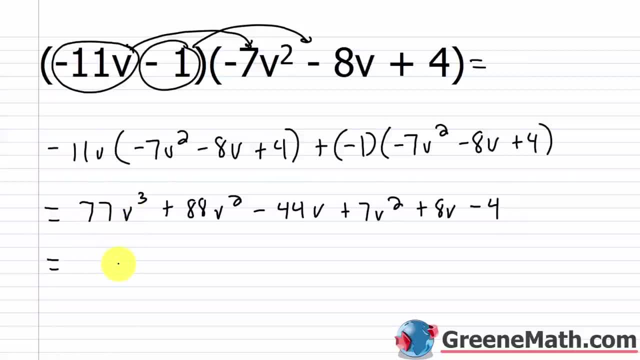 Alright, so now let's look for a like term. So 77v cubed. Nothing I can combine with that. 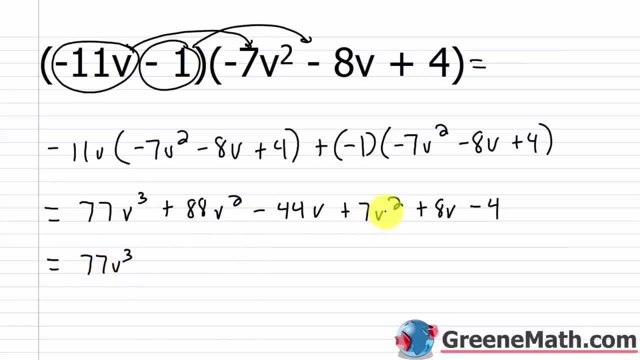 88v squared and 7v squared. Those are like terms. These are like terms. So what is 88 plus 7? Well, that's 95. 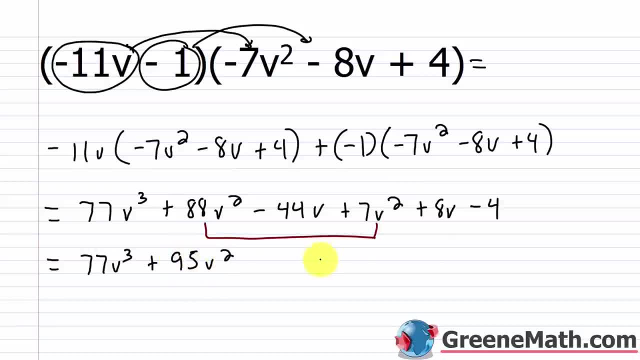 So then plus 95v squared. And then for other like terms, we have negative 44v and 8v. 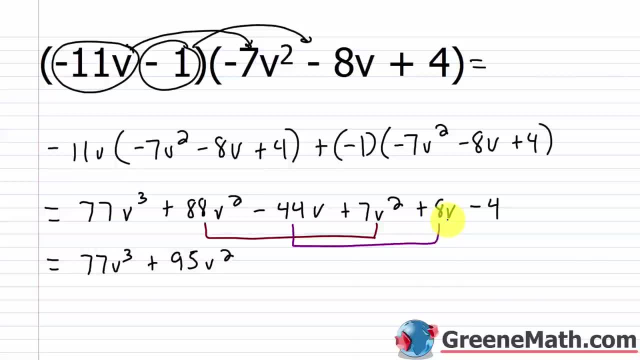 Those are like terms. So if we can combine those, you'd end up with negative 36v. 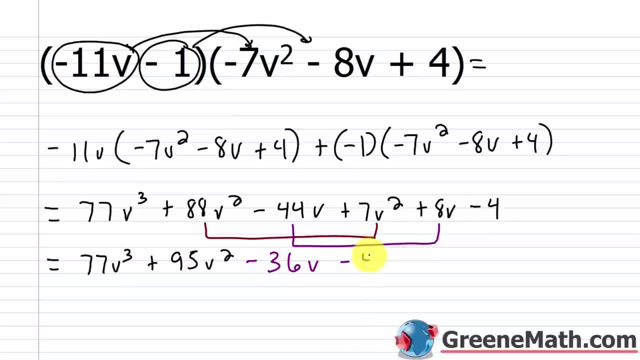 So minus 36v. And then lastly, minus 4. So we end up with 77v cubed plus 95v squared minus 36v minus 4. 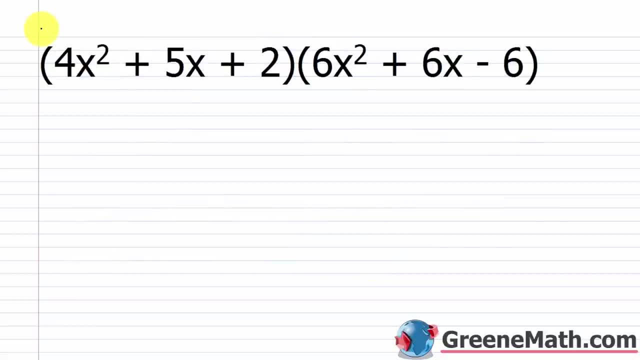 Alright, let's take a look at the next one. So now we have a trinomial times another trinomial. So this isn't getting more difficult. It's just becoming more and more tedious, right? As you expand these things out and get, you know, polynomials with more and more terms, this just becomes more tedious and harder to keep track of, you know, kind of where everything is. 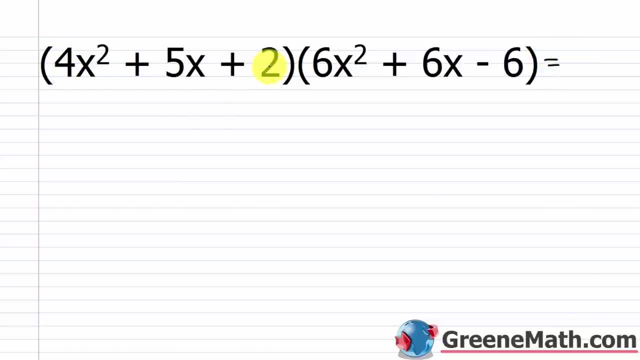 Alright, so again, I'm just going to multiply every term of the first polynomial by every term of the second polynomial. That's all I'm doing. 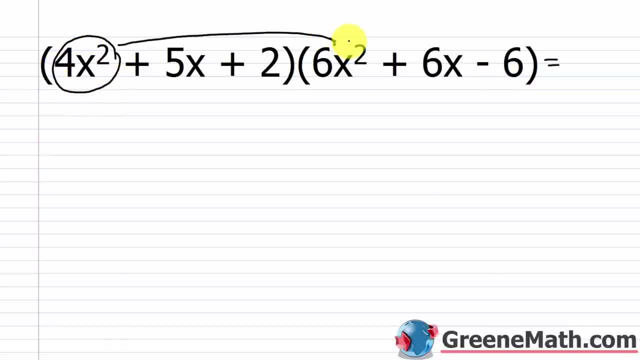 So I'm going to take 4x squared and I'm going to multiply it by this polynomial here, 6x squared plus 6x minus 6. 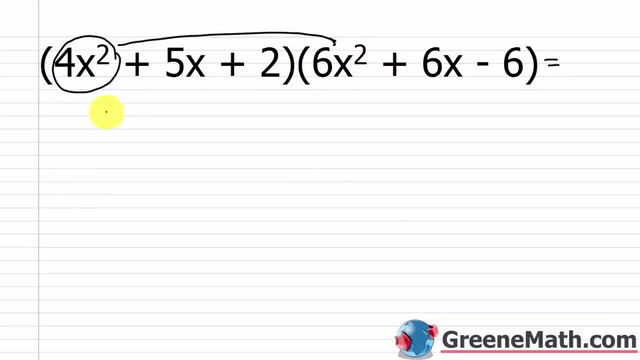 So without going through and kind of creating all this, you know, kind of extra work, let's just do it and write our answer here. So 4x squared times 6x squared. 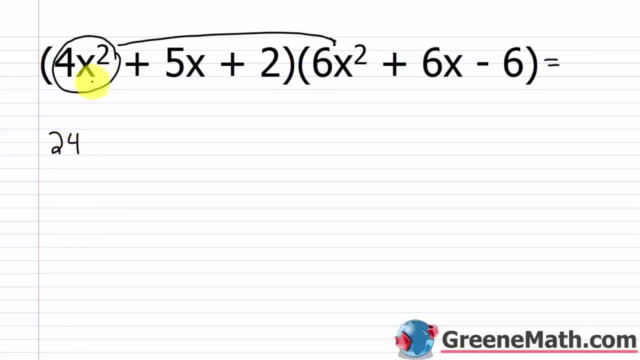 4 times 6 is 24. x squared times x squared is x to the fourth power, right? x is the base. That's common. So that stays the same. You add your exponents. 2 plus 2 is 4. 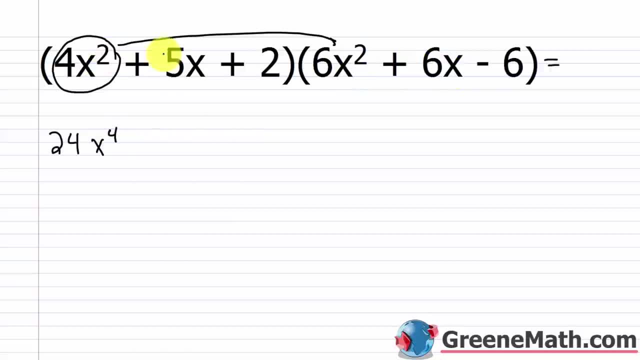 Next, I'd have 4x squared times 6x. So 4 times 6 is 24, so plus 24. x squared times x, remember this is x to the first power. So x squared times x is x cubed. Then next I have 4x squared times negative 6. 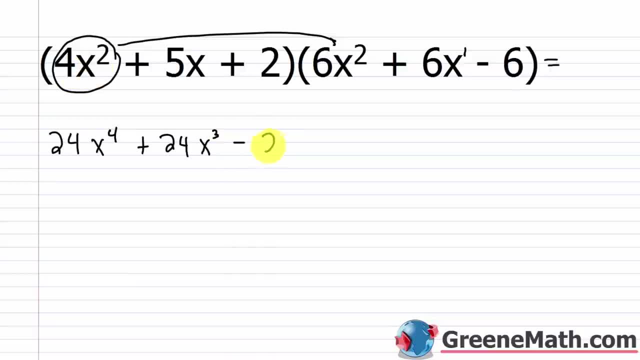 So that's going to be minus. And then 4 times 6 is 24. And then x squared. All right, so we're done with that one. 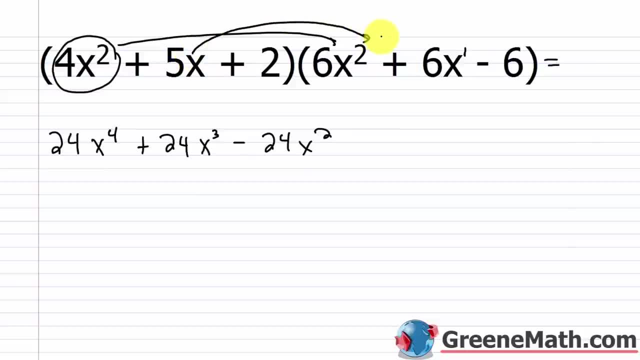 Now we're going to do 5x times this guy. So 5x times 6x squared is going to be what? 5 times 6 is 30. So plus 30. x times x squared is x cubed. 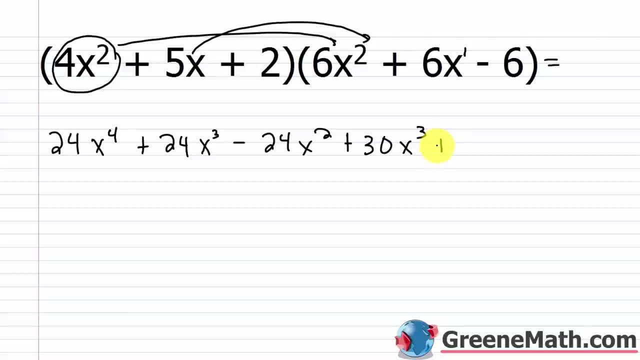 Then 5x times 6x is 30x squared. So plus 30x squared. 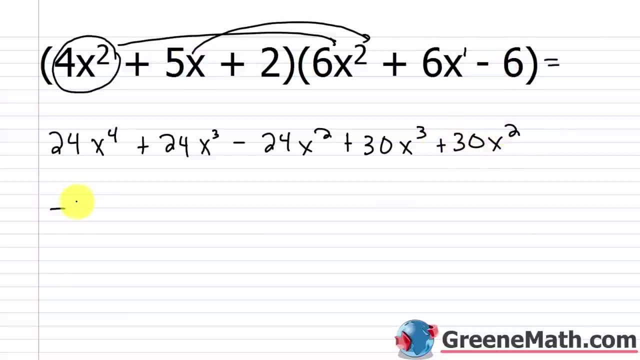 And 5x times negative 6 would be minus 30x. 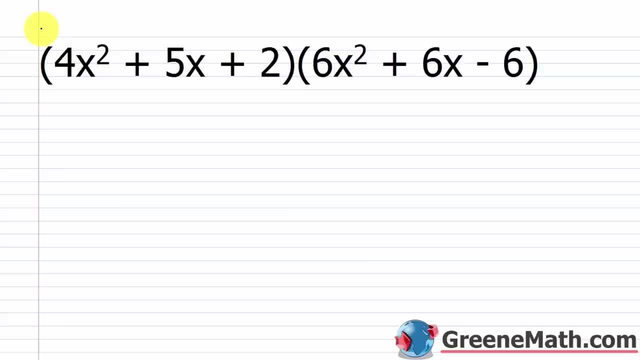 a look at the next one. So now we have a trinomial times another trinomial. So this isn't getting more difficult, It's just becoming more and more tedious, Right as you expand these things out and get you know polynomials with more and more terms, This just 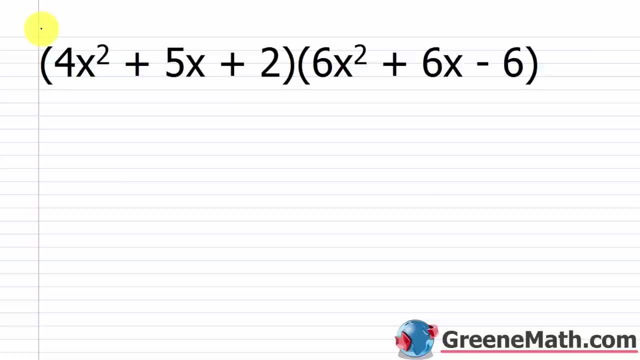 becomes more tedious and harder to keep track of. you know kind of where everything is All right. so again, I'm just going to multiply every term of the first polynomial by every term of the second polynomial. That's all I'm doing. So I'm going to take 4x squared and I'm going to multiply it by. 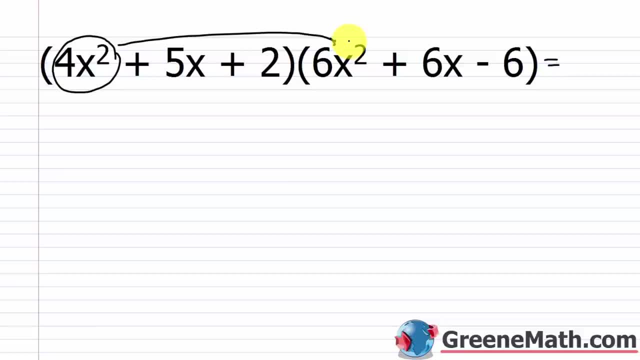 this polynomial here: 6x squared plus 6x minus 6.. So, without going through and kind of creating a all this, you know, kind of extra work, Let's just do it and write our answer here. So 4x squared times 6x squared 4 times 6 is 24.. x squared times x squared is x to the fourth power Right, x is the. 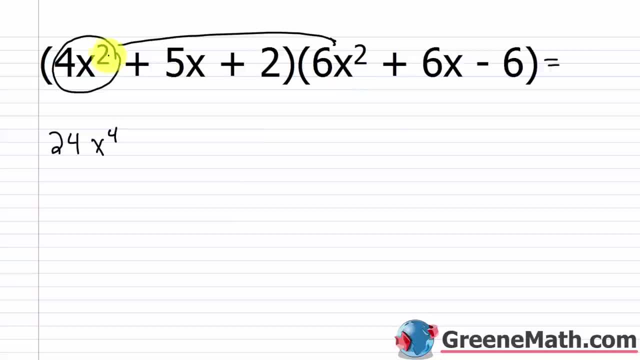 base. That's common, So that stays the same. You add your exponents: 2 plus 2 is 4.. Next I'd have 4x squared times 6x. So 4 times 6 is 24.. So plus 24.. x squared times x- Remember, this is x to the. 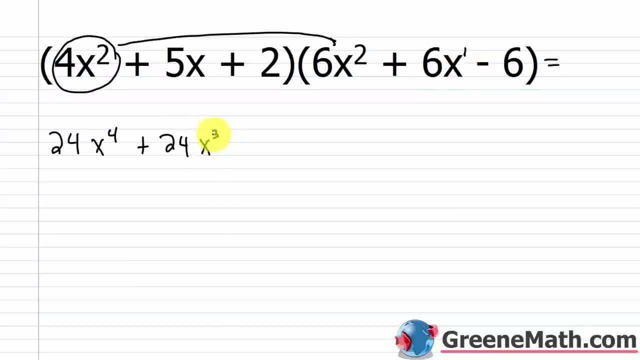 fourth power. So x squared times x is x cubed. Then next I have 4x squared times negative 6. So that's going to be minus, And then 4 times 6 is 24.. And then x squared. All right, so we're done. 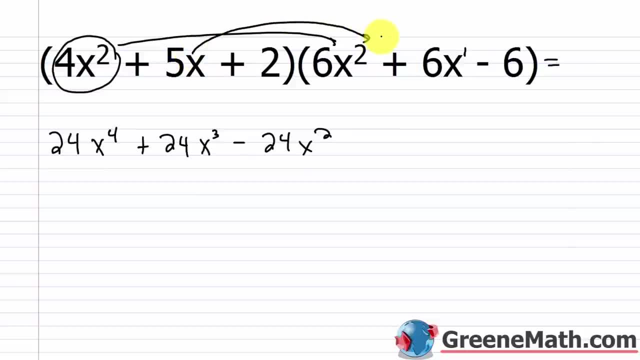 with that one. Now we're going to do 5x times this guy. So 5x times 6x squared is going to be what? 5 times 6 is 30. So plus 30. x times x squared is x cubed. Then 5x times 6x is 30x squared. 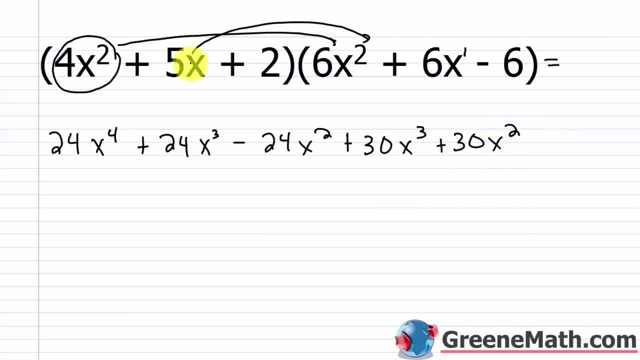 So plus 30x squared And 5x times negative 6 would be minus 30x. All right, lastly, I'm going to do 2 times this polynomial. So 2 times 6x squared is 12x squared. So plus 12x squared 2 times 6x is: 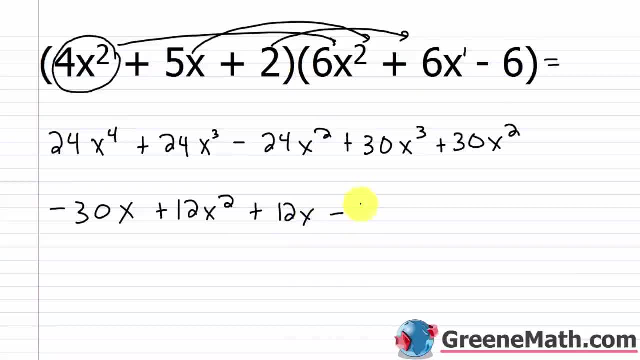 plus 12x And then 2 times negative. 6 is minus 12.. So again, it starts to become just more and more tedious. Right, it's not necessarily harder, It's just now. I got a lot of stuff that I got to. 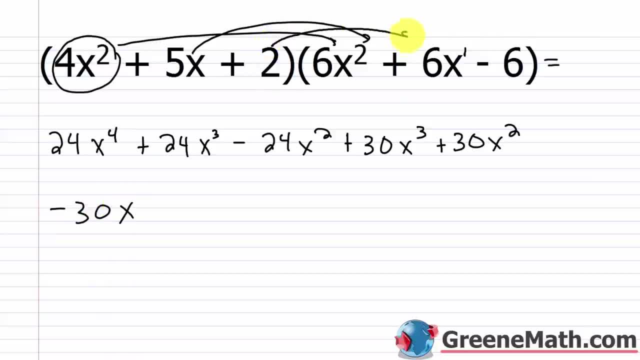 All right, lastly, I'm going to do 2 times this polynomial. So 2 times 6x squared is 12x squared. So plus 12x squared. 2 times 6x is plus 12x. And then 2 times negative 6 is minus 12. So again, it starts to become just more and more tedious, right? It's not necessarily harder. 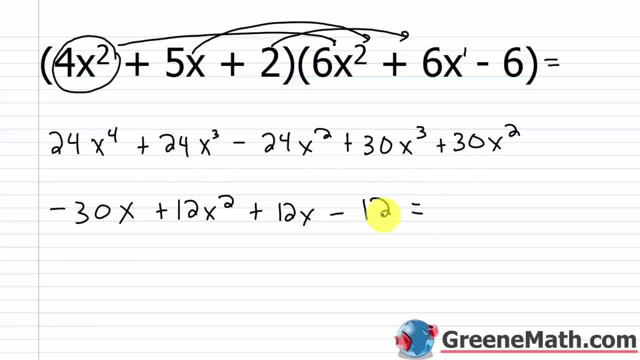 It's just now I've got a lot of stuff that I've got to keep track of. So 24x to the fourth power, nothing I can combine with that. I'm just going to rewrite that here. 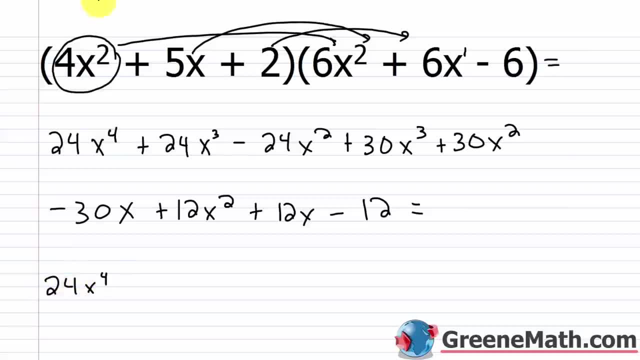 24x to the fourth power. Then I have some like terms here. So I have 24x cubed and 30x cubed. 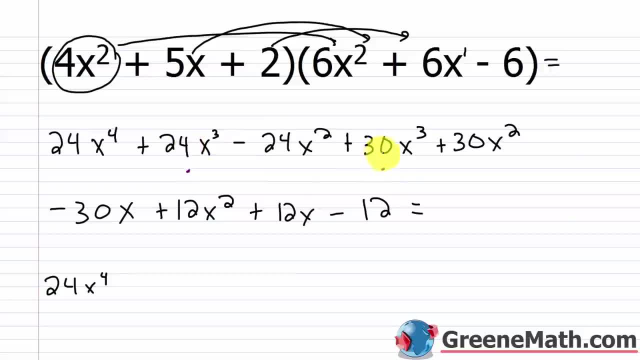 Nothing else to combine with that. So 24 plus 30 is 54. 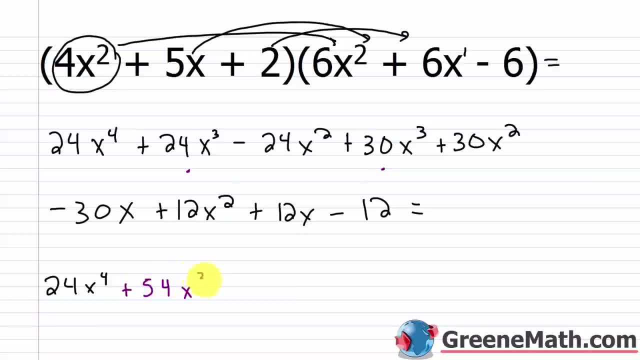 So this would be plus 54x cubed. 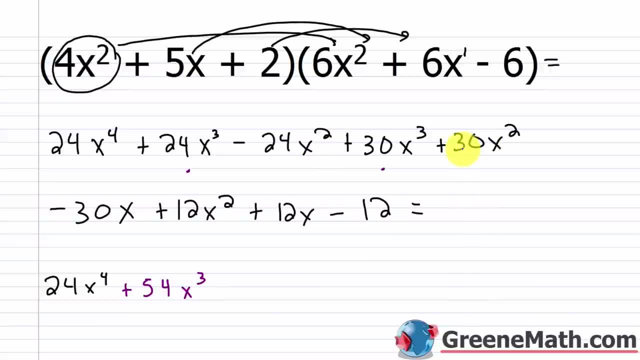 And then next I have negative 24x squared. I have 30x squared. And I have 12x squared. So these are all like terms. These are all like terms. So what is? 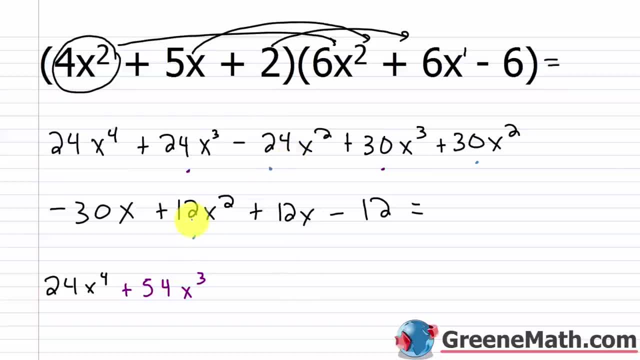 Negative 24 plus 12. Well, I know that's negative 12. And then if I had negative 12 and I had 30, that's going to give me positive 18. 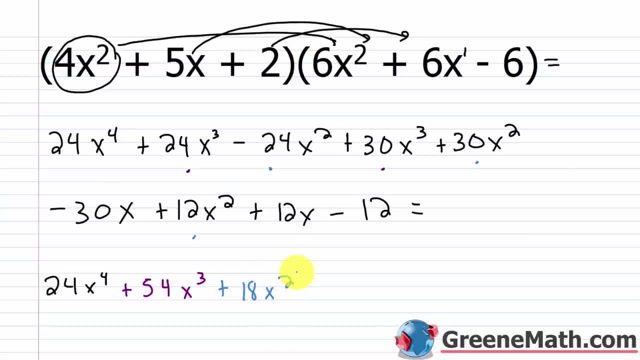 So this would be plus 18x squared. Now, I've used all of these. So now I just have, let me mark this in a different color, negative 30x and 12x as like terms. So negative 30x plus 12x is negative 18x. And then lastly, I have minus 12. Nothing to combine with that. 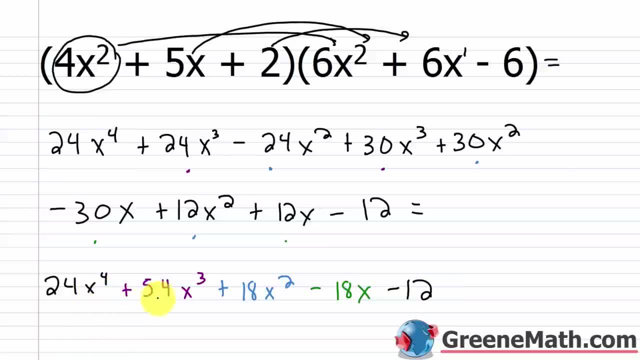 So as my answer here, I get 24x to the fourth power plus 54x cubed plus 18x squared minus 18x minus 12. 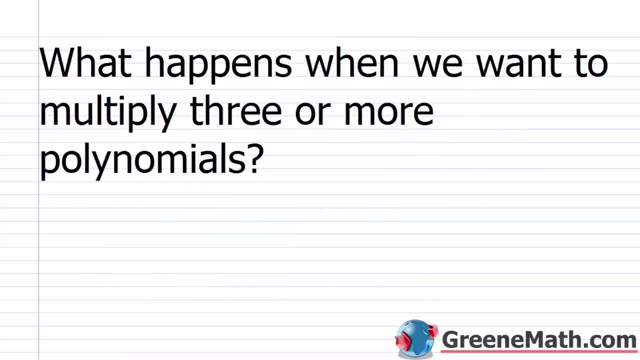 So what happens when we want to multiply three or more polynomials? Well, it's just like when you're multiplying three numbers. 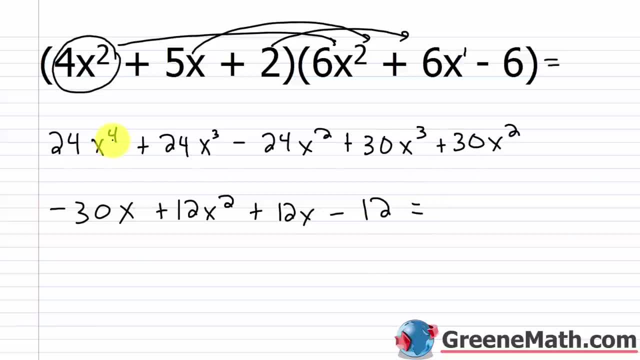 keep track of. So 24x to the fourth power, Nothing I can combine with that. I'm just going to rewrite that here. 24x to the fourth power, Then I have some like terms here. So I have 24x cubed and 30x. 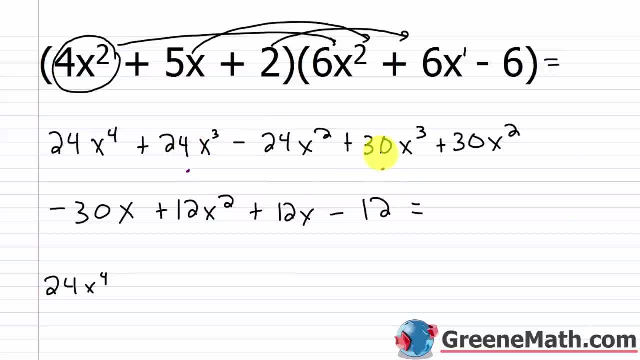 cubed, Nothing else to combine with that. So 24 plus 30 is 54.. So this would be plus 54x cubed. And then next I have negative 24x squared, I have 30x squared And I have 12x squared. 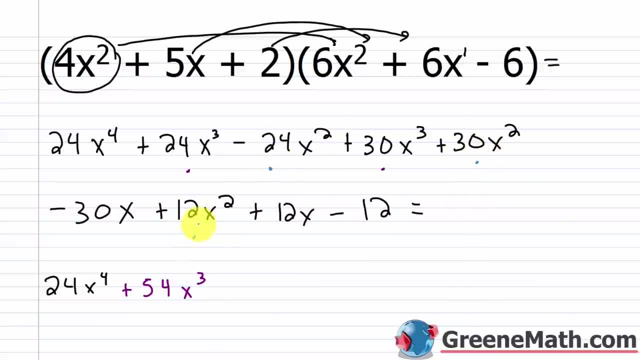 So these are all like terms. These are all like terms. So what is negative? 24 plus 12?? Well, I know, that's negative 12.. And then if I had negative 12 and I had 30, that's going to give me positive 18.. 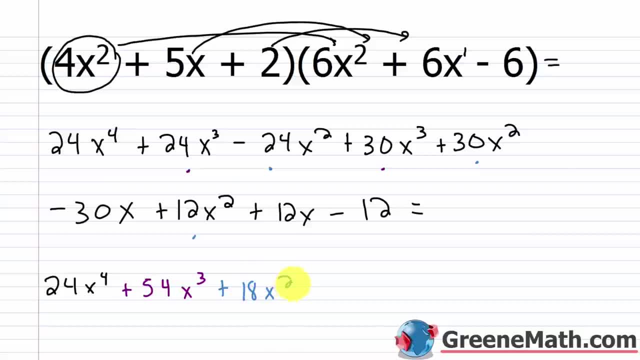 So this would be plus 18x squared. Now I've used all of these, So now I just have- let me mark this in a different color- negative 30x and 12x as like terms. So negative 30x plus. 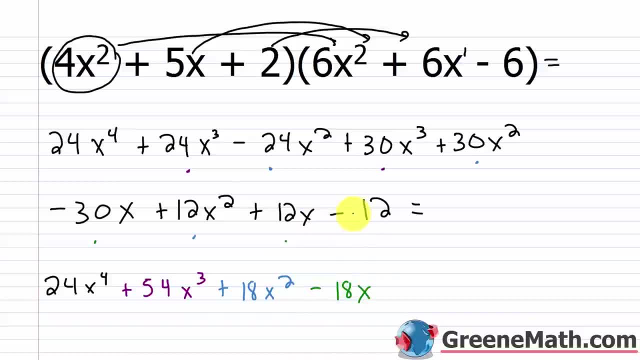 12x is negative 30x squared. So I have negative 30x squared. So I have negative 30x squared. 12x is negative 18x. And then, lastly, I have minus 12.. Nothing to combine with that. 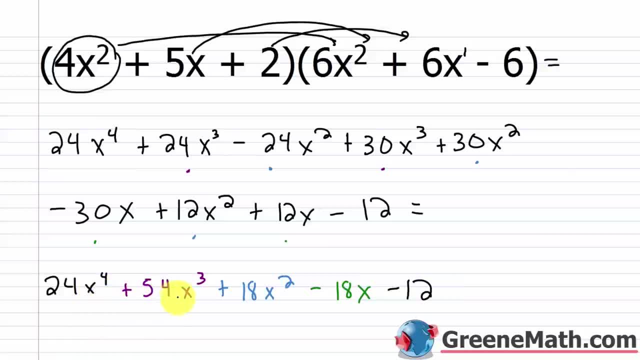 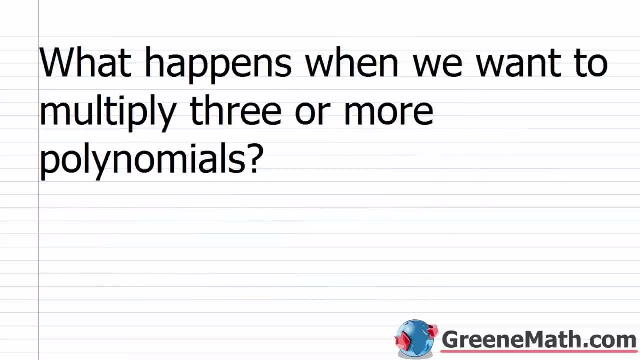 So, as my answer here, I get 24x to the fourth power plus 54x cubed, plus 18x squared, minus 18x minus 12.. So what happens when we want to multiply three or more polynomials? Well, it's just like when you're multiplying three numbers. If I have something like: 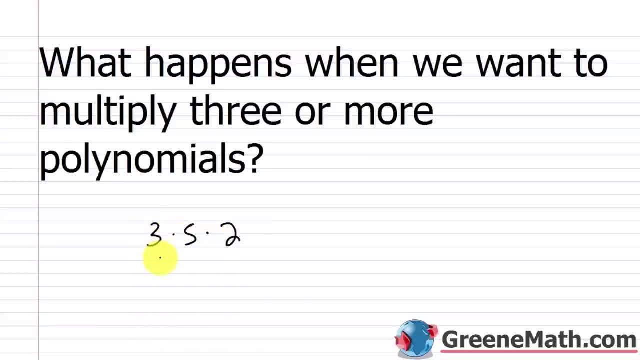 3 times 5 times 2,. I can multiply in any order, as long as I multiply everything together. So in other words, I can do 3 times 5 times, 3 times, 5 times, 2 times, 3 times, 5 times, 2 times 5 times 2 times. 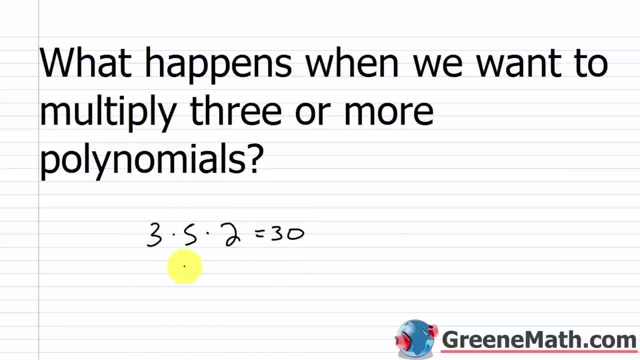 that's 15. then 15 times 2 is 30. or I could switch this up and say: okay, I can do 3 times 2 times 5. so 3 times 2 is 6, 6 times 5 is 30, or I could do it as 5 times 2 times 3. that's another way to do. 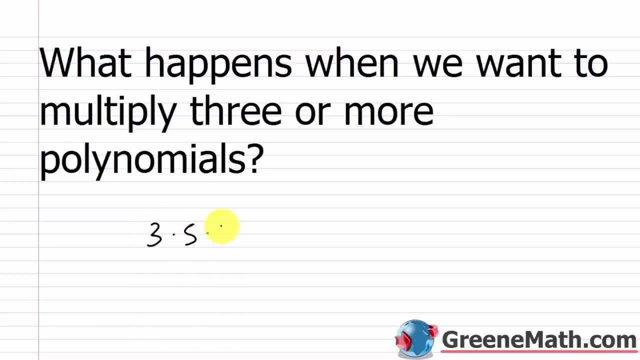 If I have something like 3 times 5 times 2, I can multiply in any order as long as I multiply everything together. So in other words, I can do 3 times 5, that's 15. Then 15 times 2 is 30. Or I could switch this up and say, okay, I can do 3 times 2 times 5. So 3 times 2 is 6. 6 times 5 is 30. 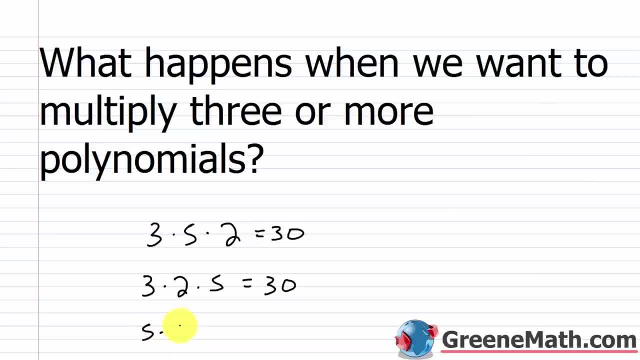 Or I could do it as 5 times 2 times 3. That's another way to do it. 5 times 2 is 10. 10 times 3 is 30. 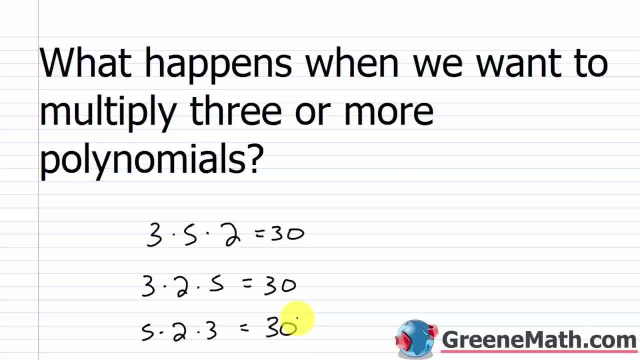 You know, as long as I multiply everything together, it doesn't really matter, the order, right? When we do multiplication, it's commutative, right? So the order is unimportant. 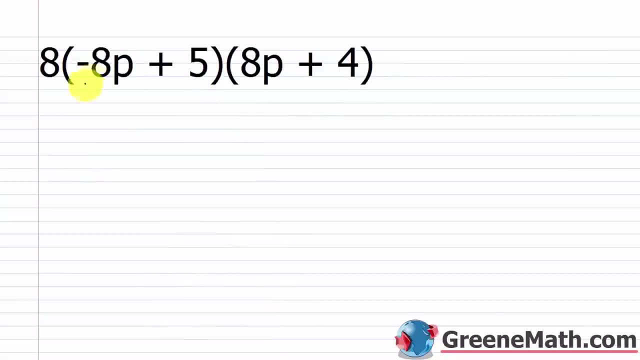 So when I look at 8 times this negative 8x. This negative 8p plus 5 times 8p plus 4. I could multiply 8 times this guy first. Or I could multiply 8 times this guy first. Or I could multiply these two guys together first. 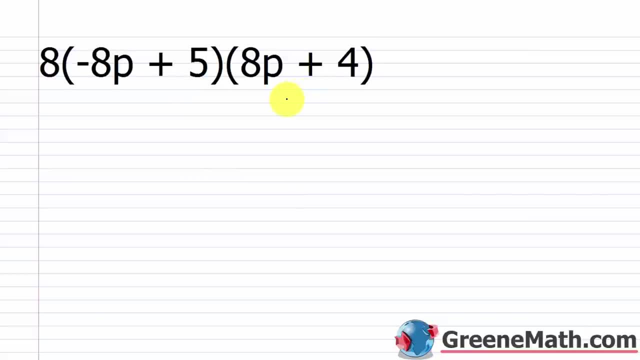 It really doesn't matter. So kind of the easiest way for me to do it, I just kind of go in order. 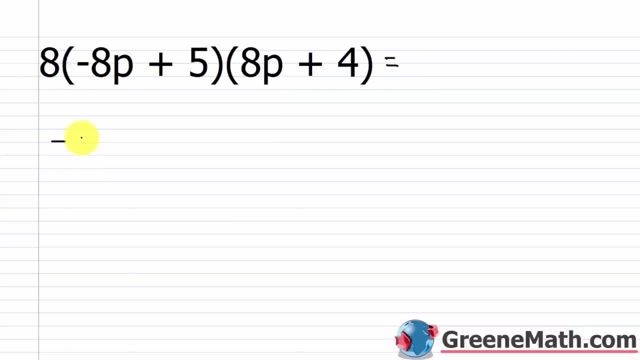 So I would start out by just saying, okay, I have 8 times negative 8p. That's negative 64p. Then I have 8 times 5. That's 40. So plus 40. So now I have this guy times this guy. And now it's a problem that's pretty easy to deal with. 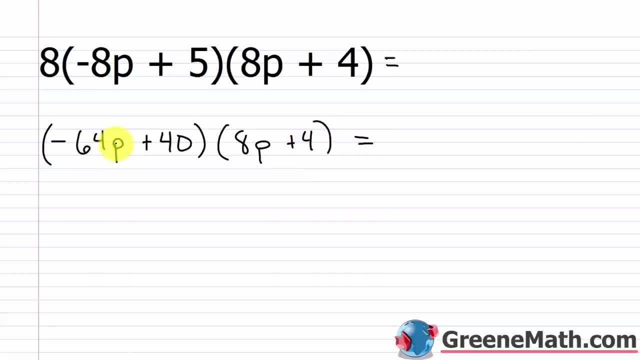 So negative 64p would be multiplied by this guy. This is going to multiply by this guy. So negative 64p times 8p. What is negative 64 times 8? We know that's negative. 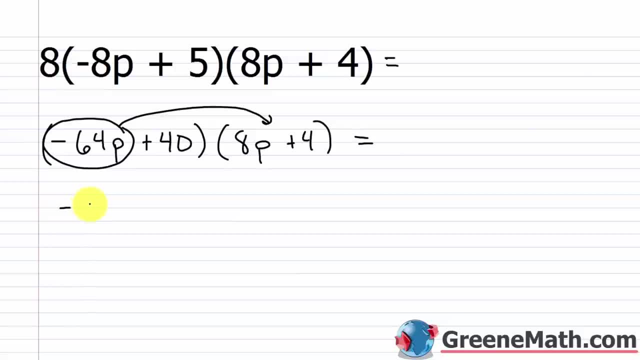 And then 64 times 8 is 512. So negative 512. 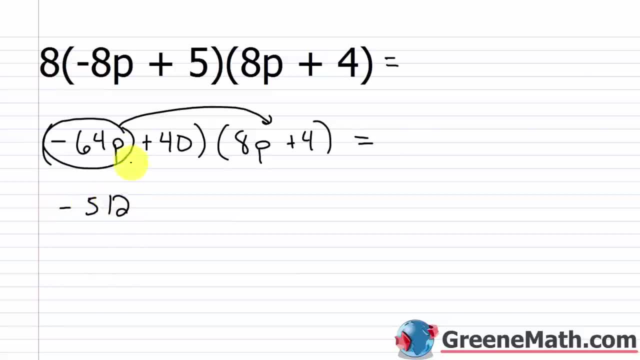 p times p is p squared. And then what is negative 64p times 4? Well, we know that's, again, negative. 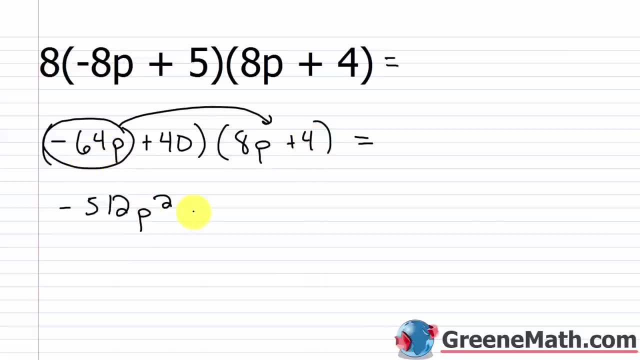 And then 64 times 4 is 12. And then what is negative 64p times 4? Well, negative 64 times 4 is 256. So negative 256p. And then we have 40 times this guy. So 40 times 8p. 4 times 8 is 32. And then put a 0 at the end. That would be 320. 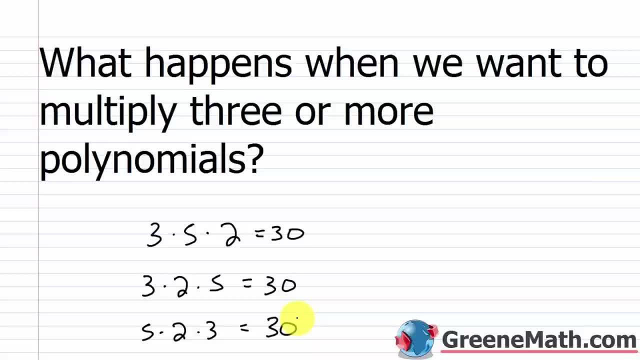 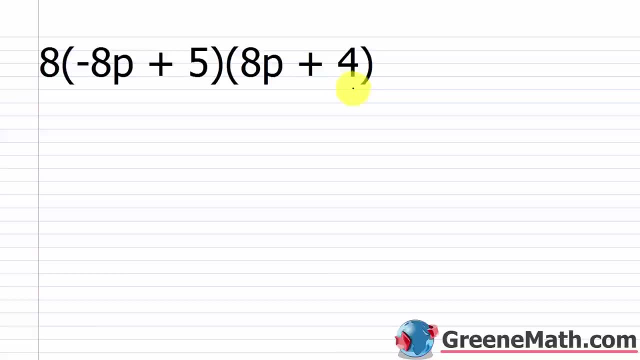 it: 5 times 2 is 10, 10 times 3 is 30. you know, as long as I multiply everything together, it doesn't really matter the order, right? when we do multiplication it's commutative, right? so the order is unimportant. so when I look at 8 times this negative 8p plus 5 times 8p plus 4, I could 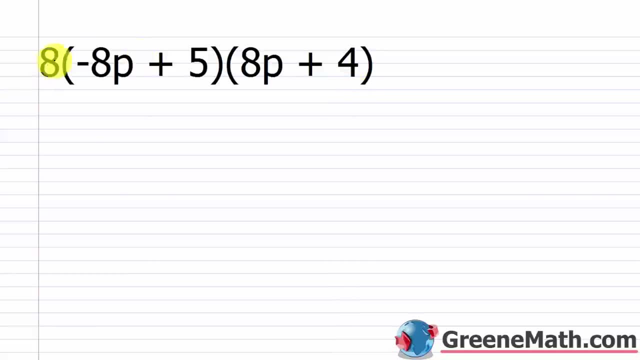 multiply 8 times this guy first, or I can multiply 8 times this guy first, or I could multiply these two guys together first. it really doesn't matter, so kind of the easiest way for me to do it. I just kind of go in order. so I would start out by just saying: okay, I have 8 times negative, 8p, that's. 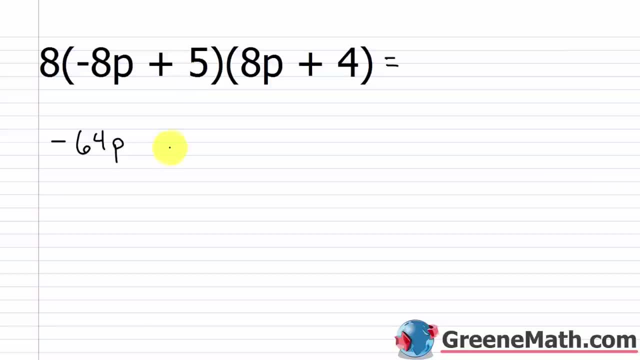 negative 64p, then I have 8 times 5, that's 40. so plus 40 you. so now I have this guy times this guy, and now it's a problem that's pretty easy to deal with. so negative 64p would be multiplied by this guy. this is going to multiply by this guy, so negative. 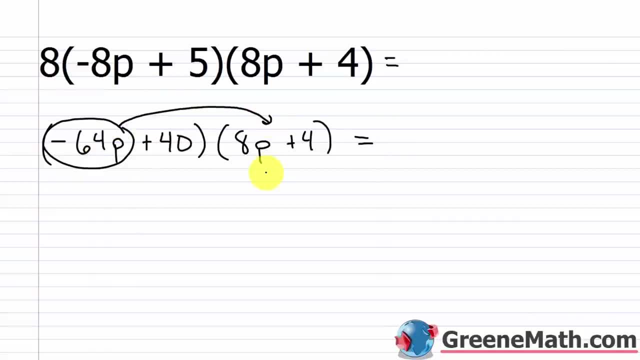 64p times 8p. what is negative? 64 times 8? we know that's negative. and then 64 times 8 is 512. so negative: 512 p times p is p squared. and then what is negative? 64p times 4? we know that's again. 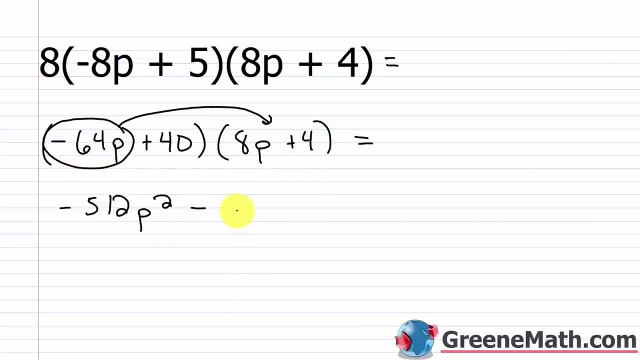 negative. we know that's again negative, so negative. 64 times 4 is positive minus 225. so negative: 6 to plus 7 in 3 times 4 plus 3. that's breaking it down on negative. and then split is equal to 0. so negative: 2, 15, 5 over 9, log negative 4 times 8 times 8 p. and then 64 times 4 is 23. 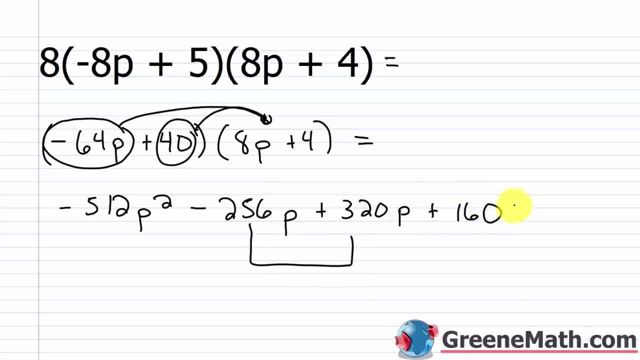 so now I can combine like terms here so I could put: negative 512 p squared negative 256 p plus 320 p is 64 p, so plus 64 p and then plus 160. so there's my answer: negative 512 p squared plus 64 p plus 160. now, if you wanted to, I'm not going to do in this video in the interest of time. 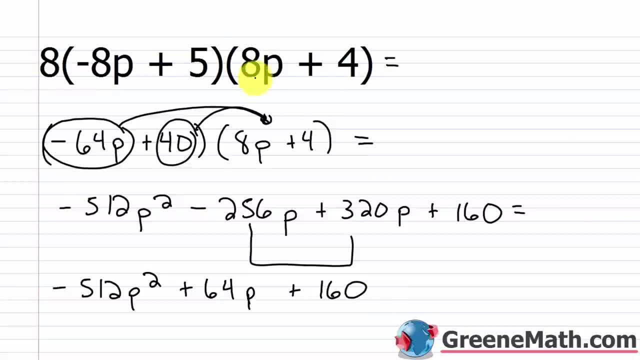 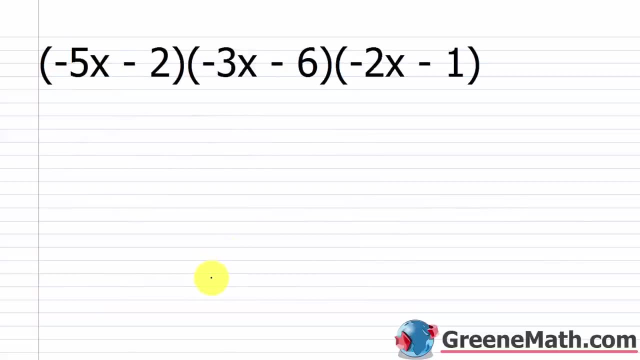 you can multiply 8 times this polynomial here, 8 p plus 4 first, then multiply that product by this guy. you're going to get the same answer either way. so the order is not important again when you're multiplying, and we know that from basic pre-algebra. all right, for the last problem. we have something. 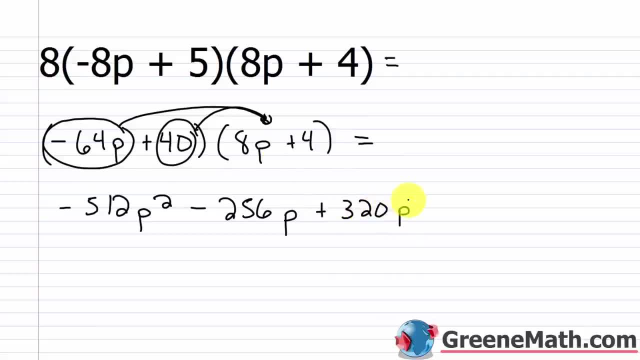 So plus 320. Don't forget about the p. And then 40 times 4. That's easy. 4 times 4 is 16. Put a 0 at the end. It's 160. So now I can combine like terms here. I put negative 512p squared. 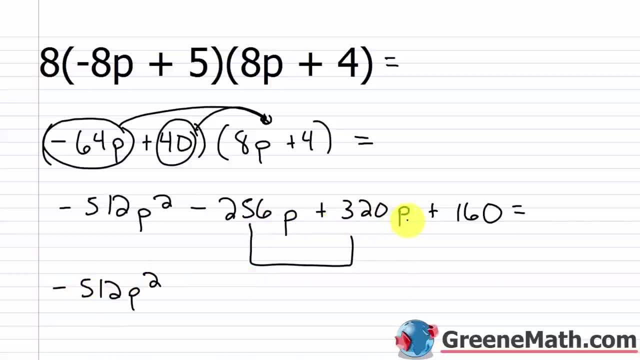 Negative 256p plus 320p is 64p. So plus 64p. And then plus 160. So there's my answer. 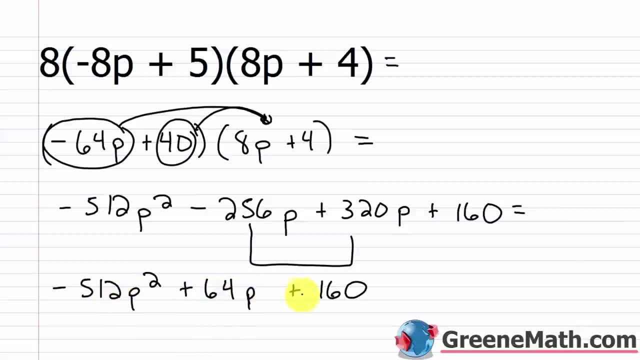 Negative 512p squared plus 64p plus 160. Now if you wanted to, I'm not going to do it in this video in the interest of time. You can multiply 8 times this polynomial here. 8p plus 4 first. Then multiply that product. By this guy. You're going to get the same answer either way. 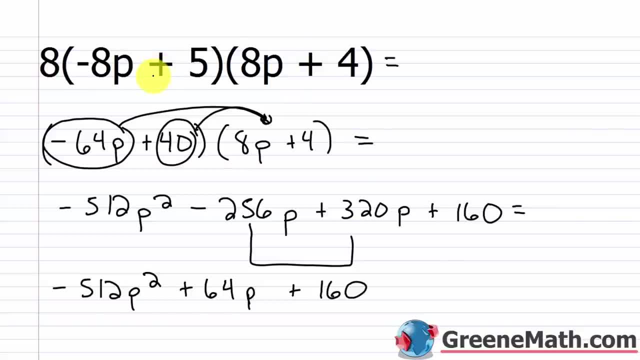 So the order is not important, again, when you're multiplying. And we know that from basic pre-algebra. All right. 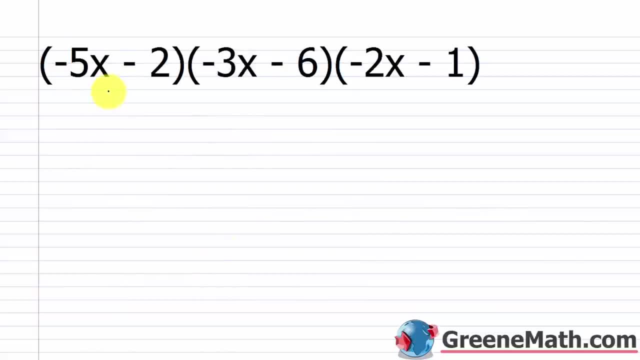 For the last problem, we have something that's going to be a little tedious. We have negative 5x minus 2 times negative 3x minus 6 times negative 2x minus 1. So again, if you're multiplying, the order isn't important. So I can go left to right. I can multiply these two together first and then multiply. 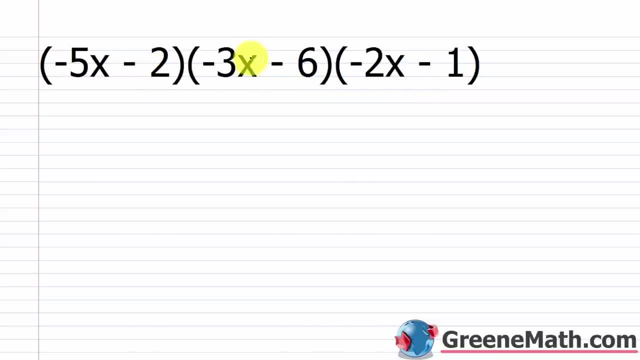 It doesn't matter. So what I like to do is just multiply these two together first. Get a product. 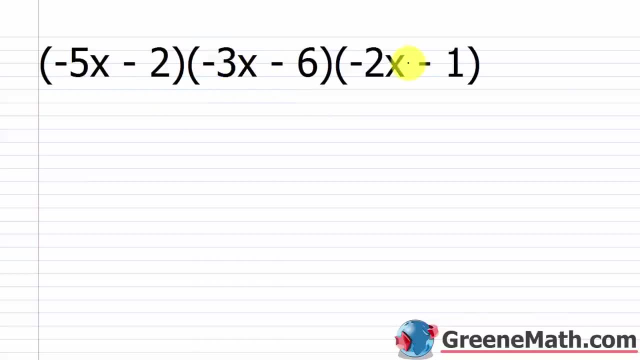 And then take that and multiply it by this. 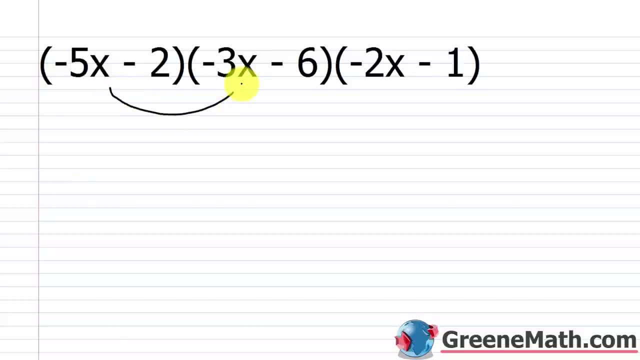 So I'm going to start out by just finding the product of these two. So if I had that problem here, I would have negative 5x times this right here. 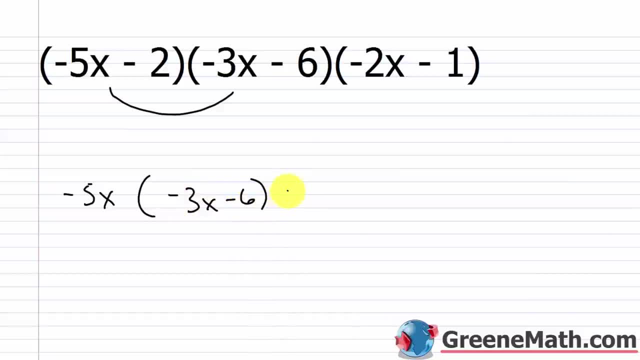 This negative 3x minus 6. And then plus, I'd have negative 2 times negative 3x minus 6. 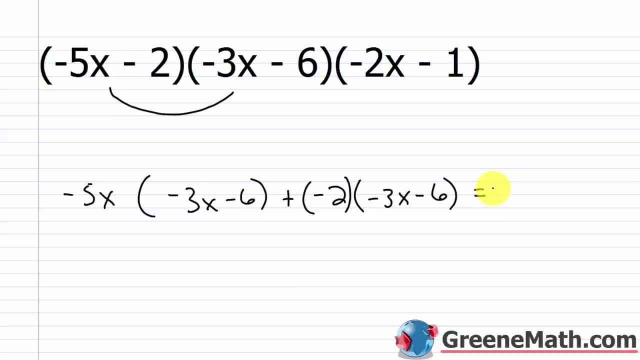 Let's figure out what that is first. So negative 5x times negative 3x. That would be plus. Plus 15x squared. Negative 5x times negative 6. That would be plus 30x. Negative 2 times negative 3x would be plus 6x. Negative 2 times negative 6 would be plus 12. So essentially what I'm transforming this problem into is this guy right here. 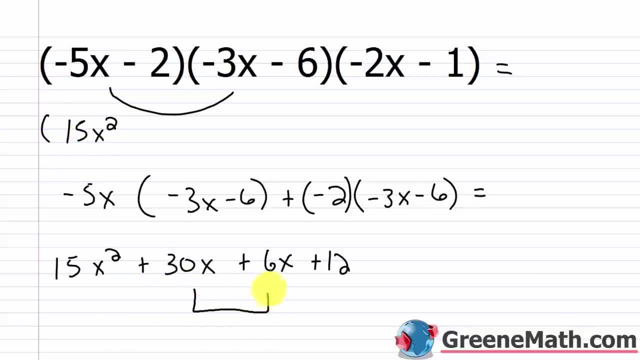 I'd have 15x squared. Combine like terms here. 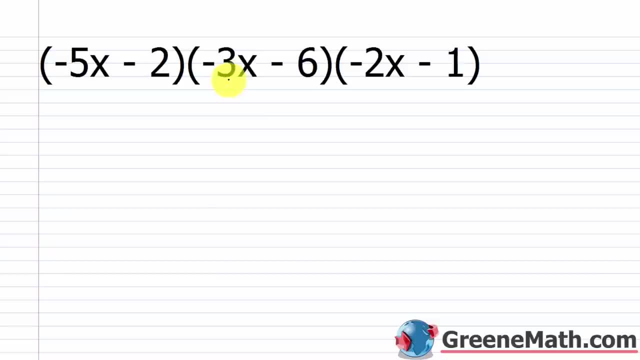 that's going to be a little tedious. we have negative 5x minus 2 times negative 3x minus 6 times negative 2x minus 1. so again, if you're multiplying, the order isn't important, so I can go left to right, I can multiply. 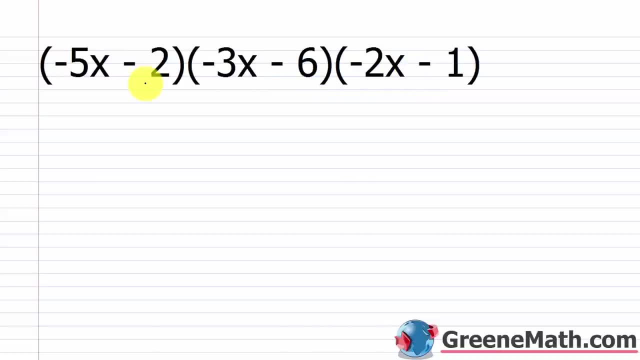 you can go left to right, I can multiply. you can go left to right, I can multiply these two together first and then multiply. it doesn't matter. so what I like to do is just multiply these two together. first get a product and then take that and multiply it by this. 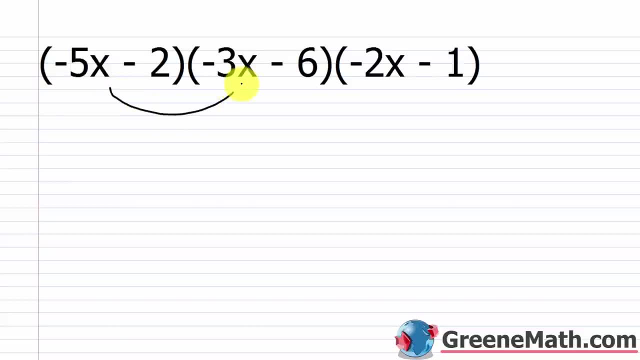 so I'm going to start out by just finding the product of these two. so if I had that problem here, I would have negative 5x times this right here, this negative 3x minus 6, and then, plus, I'd have negative 2 times negative 3x minus 6. 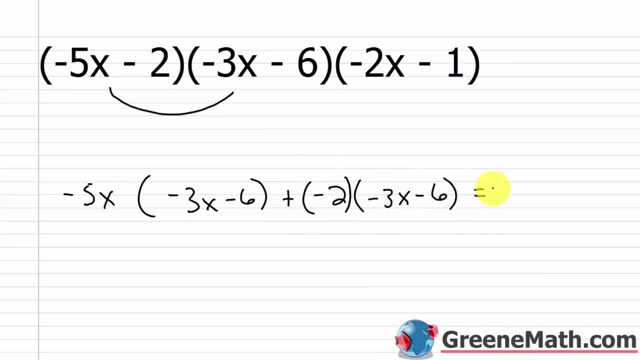 let's figure out what that is first. so negative 5x times negative: 3x- that would be plus 15x squared. negative 5x times negative: 6- that would be plus 30x. negative 2 times negative: 3x would be plus. 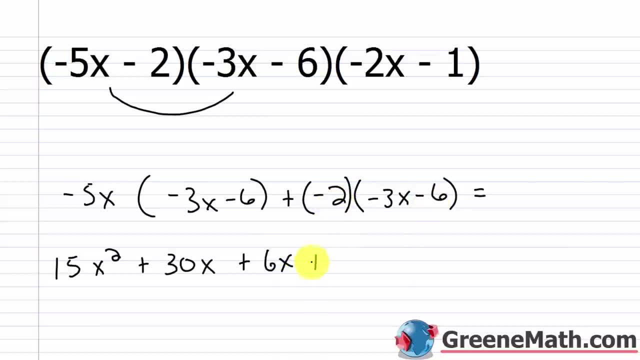 6x negative, 2 times negative, 6 would be plus 12. so essentially, what I'm transforming this problem into is this guy right here, I'd have 15x squared combined with this guy right here, I'd have 15x squared combined with this guy right here, I'd have 15x squared combined with this guy. this like terms here: 30x. 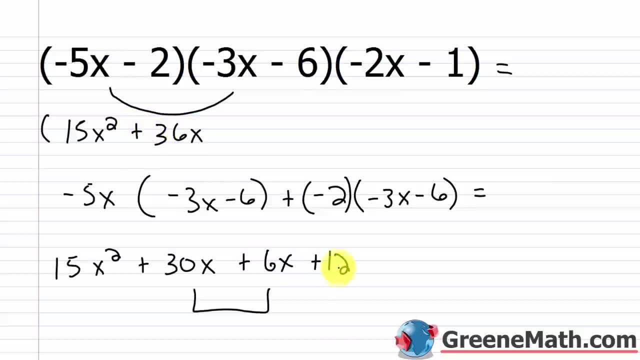 here: 30x plus 6x is plus 36x, and then plus 12 times this guy, this negative 2x minus 1. so an easy way to think about the step that we're at now. if I had 3 times 2 times 5, well, I. 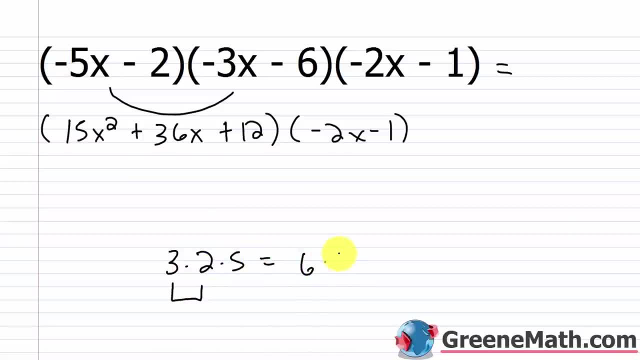 would do these two first if I wanted to. 3 times 2 is 6, I'd have 6 times 5. now that's exactly what I did here: multiply these 2 together first, and now I have that product here times this kind of last one. so now I have this. 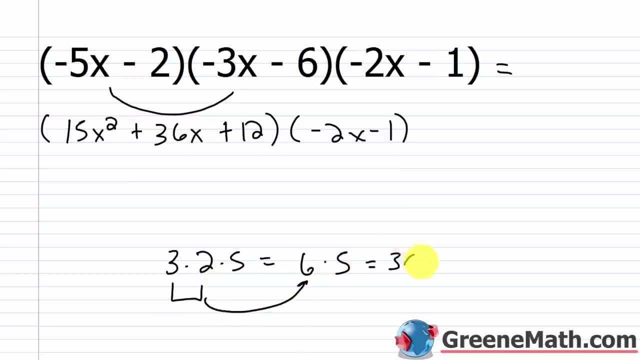 here times this kind of last one here. so the end result is 30 and again you can switch the order around if you want. it doesn't matter, you're gonna put the same result. so now I got to take each term of this first polynomial multiply by each. 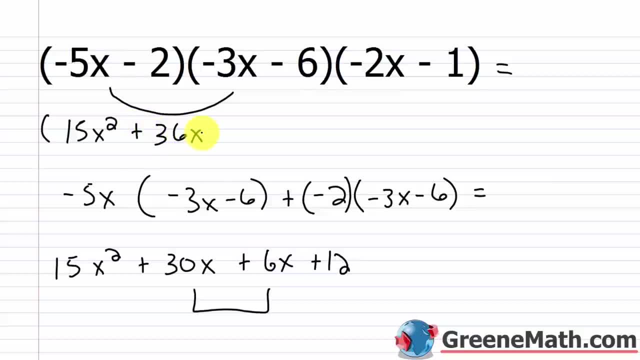 30x plus 6x is plus 36x. And then plus 12 times this guy. This negative 2x minus 1. 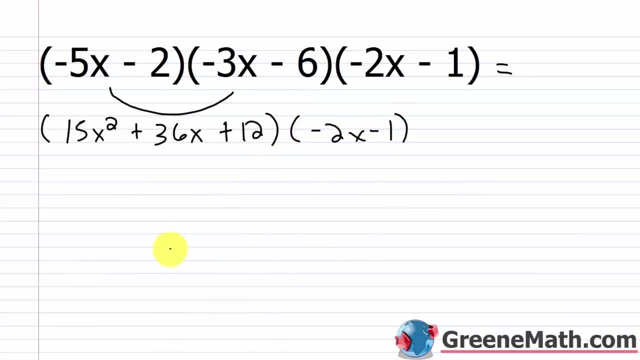 So an easy way to think about the step that we're at now, if I had 3 times 2 times 5, well I would do these two first if I wanted to. 3 times 2 is 6. I'd have 6 times 5 now. 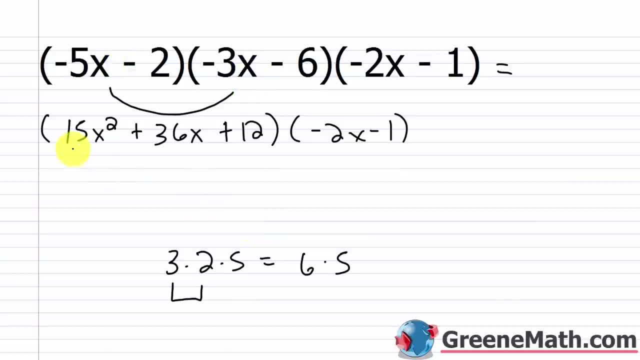 That's exactly what I did here. I multiplied these two together first. And now I have that product here times this kind of last one. So now I have this product here times this kind of last one here. So the end result is 30. 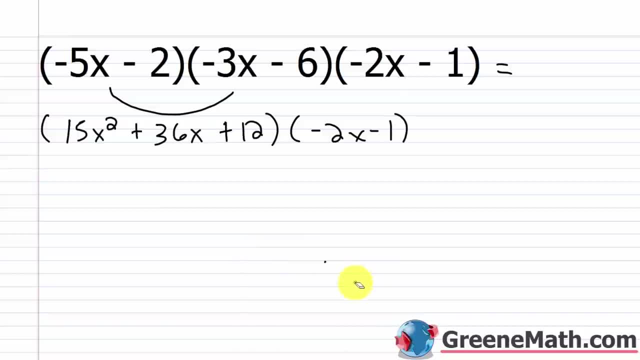 And again, you can switch the order around if you want. It doesn't matter. You're going to end up with the same result. 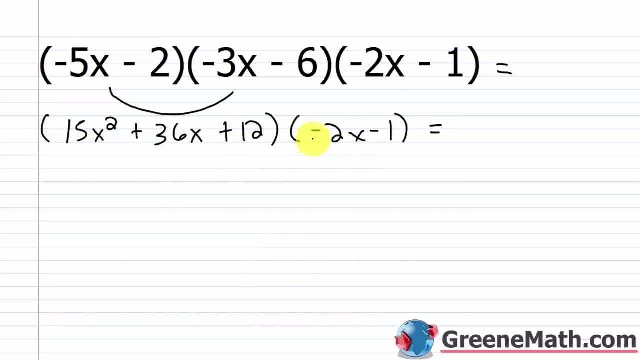 So now I've got to take each term of this first polynomial, multiply it by each term of the second polynomial. 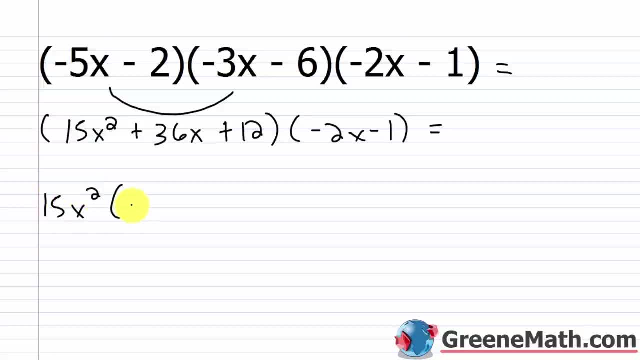 So I'm going to do 15x squared times this negative 2x minus 1. And then plus, I'm going to have 36x times this negative 2x minus 1. And then plus, I'm going to have 12 times this negative 2x minus 1. All right. 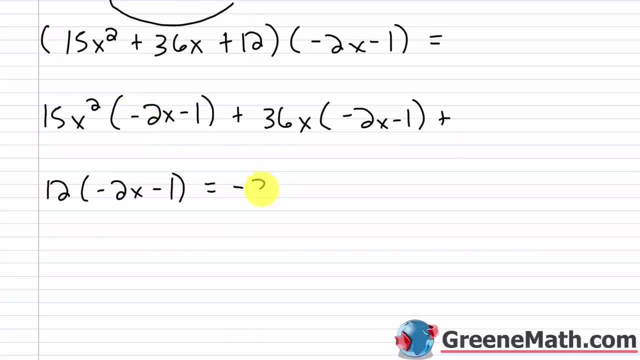 So 15x squared times negative 2x, that's going to give me negative 30x cubed. Then 15x squared times negative 1 is negative 15x squared. Then 36x times negative 2x is going to be negative 72x squared. Then 36x times negative 1 is going to be negative 36x. And then lastly, I have 12 times negative 2x. 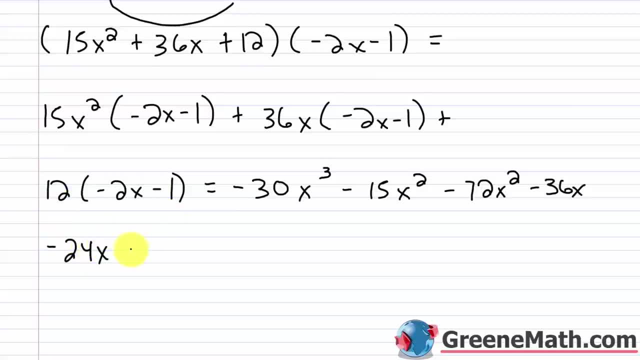 That's minus 24x. And then 12 times negative 1 is negative 12. So combine like terms here. I have negative 30x cubed. I have negative 15x squared and negative 72x squared. That's going to give me negative 87x squared. And then I have negative 36x minus 24x. That's going to be negative 60x. And then lastly, minus 12. 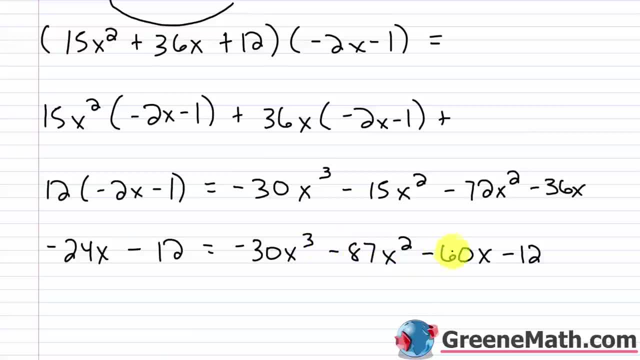 So we end up with negative 30x cubed minus 87x squared minus 60x minus 12. 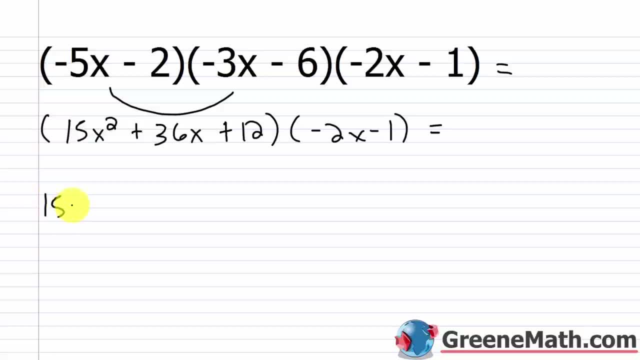 term of the second polynomial. so I'm gonna do 15x squared times this negative 2x minus 1, and then plus I'm gonna have 36x times this negative 2x minus 1, and then plus I'm gonna have 12 times this negative 2x minus 1. all right, so 15x. 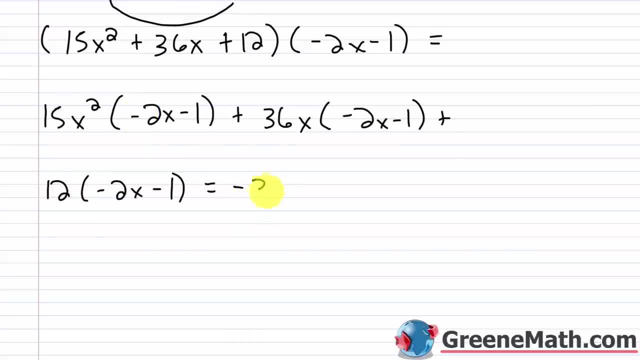 squared times negative: 2x, that's gonna give me negative 30x cubed. then 15x squared times negative: 1 is negative. 15x squared, then 36x times negative: 2x is gonna be negative. 72x squared, then 36x times negative: 1 is gonna be negative. 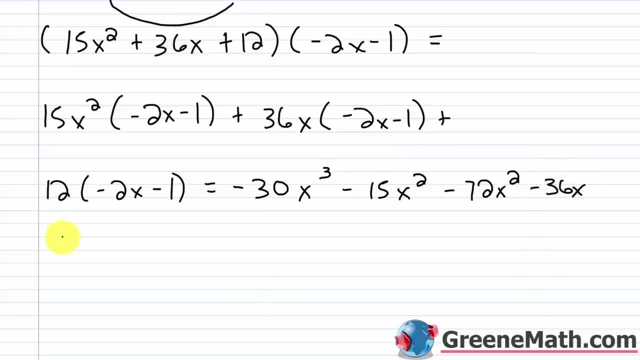 36x. and then, lastly, I have 12 times negative 2x, that's minus 24x. and then 12 times negative 1 is negative 12. so combine like terms. here I have negative 30x cubed, I have negative 15x squared and negative 72x squared. that's gonna give me. 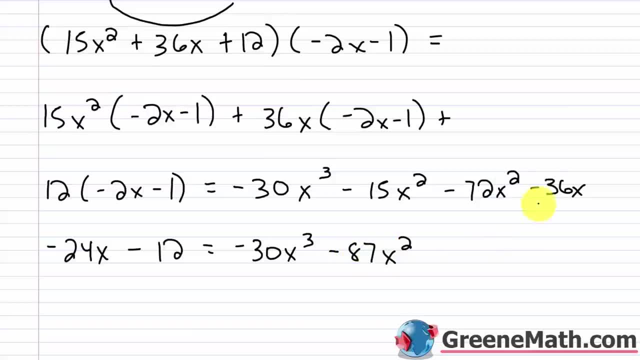 negative 87x squared, and then I have negative 36x minus 24x, that's gonna be negative 60x and then lastly minus 12. so when up with negative 30x cubed minus 87x squared, minus 60x minus 12, hello. 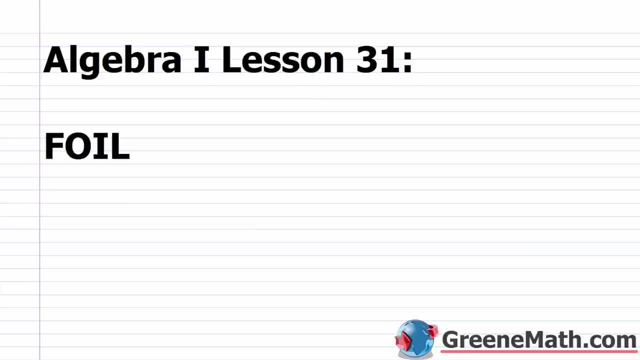 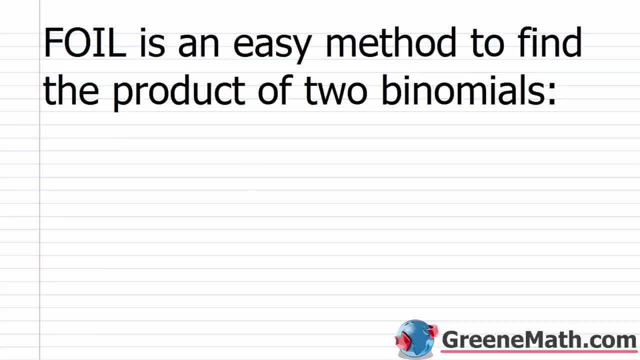 and welcome to algebra 1, lesson 31. in this video we're gonna learn about foil, alright, so in the last lesson we learned all about how to multiply 2 or more polynomials together. now in this lesson we're gonna focus specifically on kind of an easy method to get the product of two binomials. so that's what Foyle MRC is. Foyle is an. 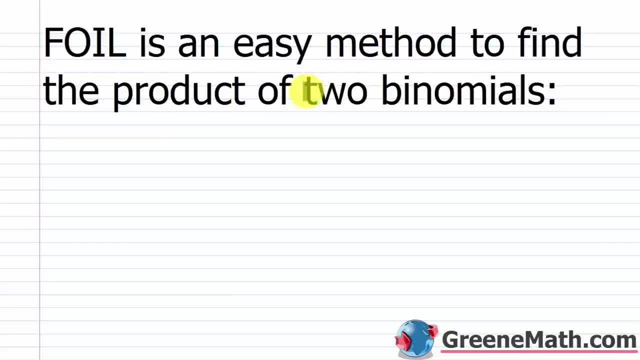 easy method to find the product of again two binomials. So it's only going to work if I have something like x plus 5 times, let's say 2x minus 1, right, Those are each binomials We multiply. 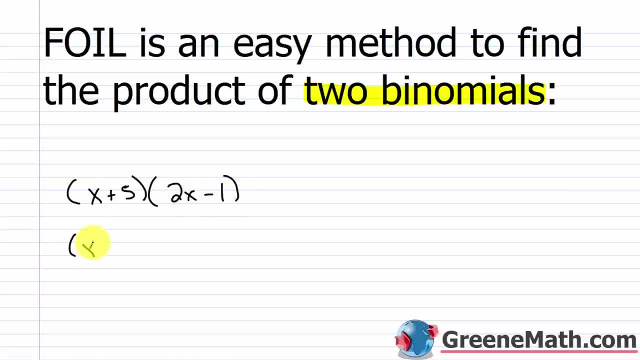 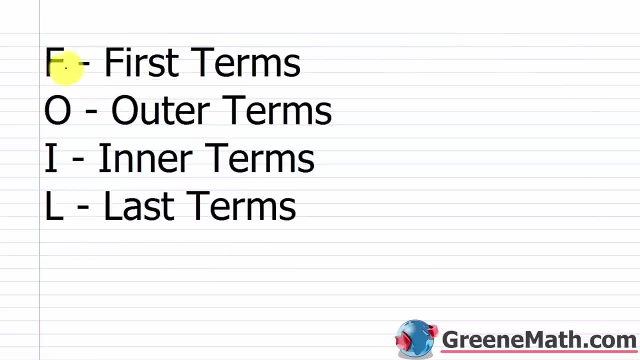 them together. We can use this FOIL, Or something like x minus 3 times x plus 2, right Two binomials being multiplied together. All right, so FOIL is an acronym And basically each letter stands for something. So the F in FOIL stands for first terms. So I'm going to start out by multiplying my first. 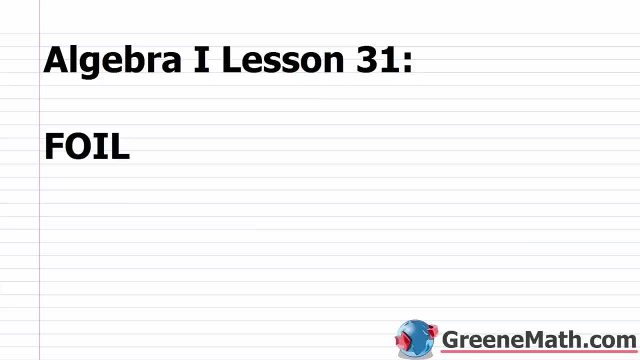 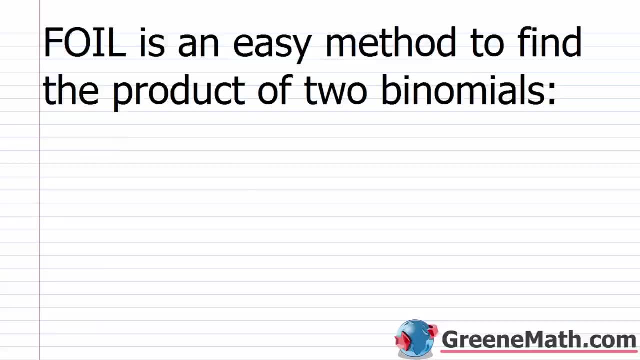 Hello and welcome to Algebra 1 Lesson 31. In this video, we're going to learn about FOIL. All right. So in the last lesson, we learned all about how to multiply two or more polynomials together. Now in this lesson, we're going to focus specifically on kind of an easy method to get the product of two binomials. So that's what FOIL is. FOIL is an easy method to find the product of, again, two binomials. So it's only going to work if I have something like this. 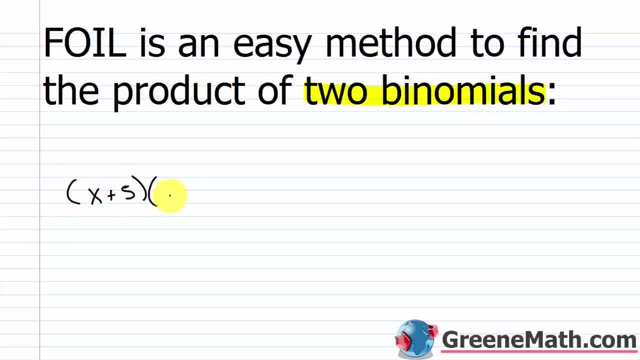 Something like x plus 5 times, let's say, 2x minus 1. All right. Those are each binomials. We multiply them together. We can use this FOIL. 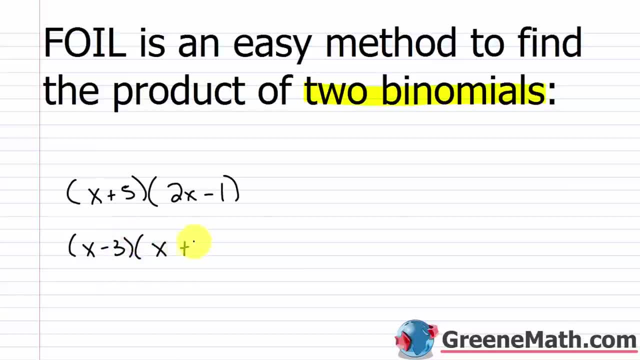 Or something like x minus 3 times x plus 2. Right? Two binomials being multiplied together. All right. 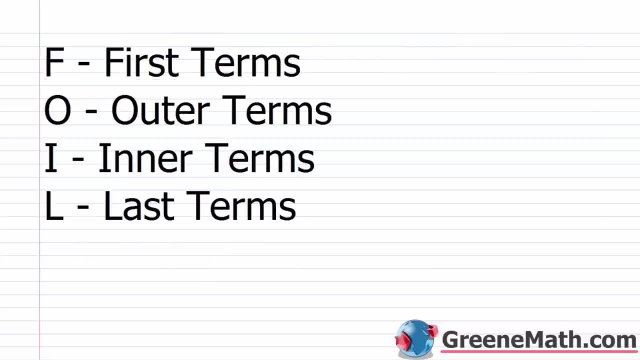 So FOIL is an acronym. And basically, each letter stands for something. So the F in FOIL stands for first terms. So I'm going to start out by multiplying my first terms together. The O stands for outer terms. So kind of my second step would be to multiply the outer terms together. The I stands for inner terms. So my third step is to multiply the inner terms together. And then the L means the last terms or the final terms. 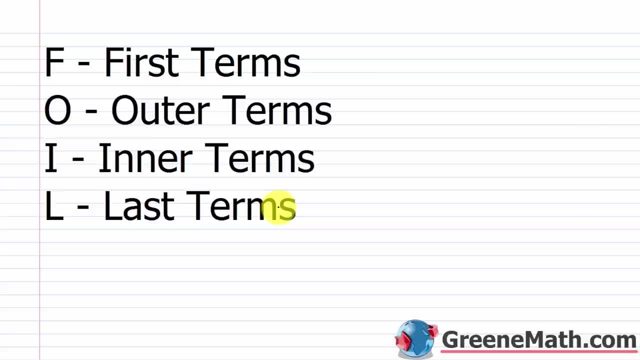 So my final step is to multiply the final terms together. 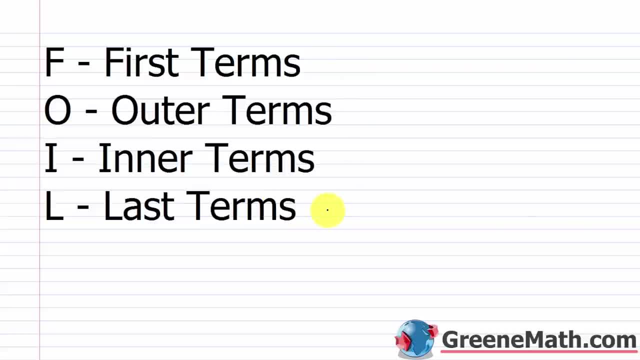 Now when you first hear about FOIL, it seems a little confusing. You're like, what are the first terms? What are the outer terms? Once you do it, let's say, 10 or 15 times, 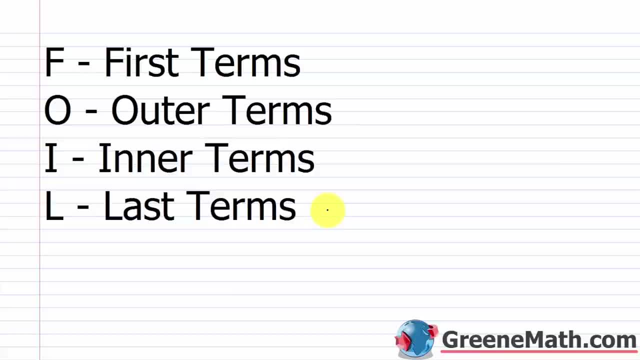 this becomes a method that you use for the rest of your life. I go through every time I multiply two binomials together. I use FOIL because it's just really, really easy to keep track of what's going on. So let's start out with this first problem. 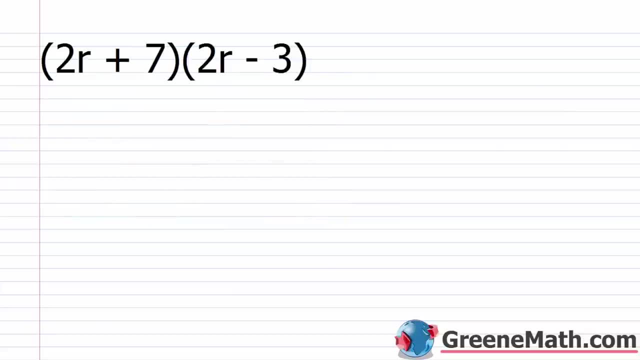 And the first way I'm going to do it is the way I showed you in the last lesson. So I have 2r plus 7 times 2r minus 3. So in the last lesson, I kind of took each term from the first polynomial and just multiplied it by the second. So I did 2r times 2r minus 3. And then plus, I would do 7 times 2r minus 3. And this is not wrong. We can still use this. So 2r times 2r is 4r squared. 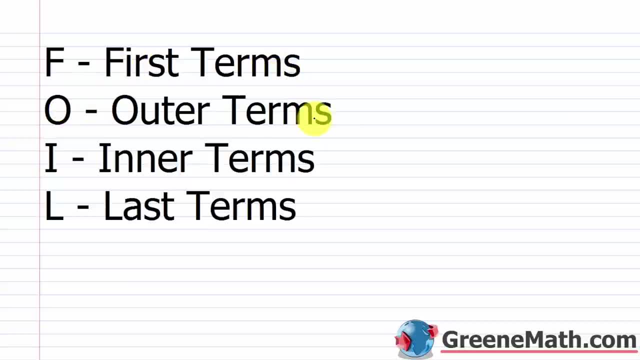 terms together. The O stands for outer terms. So kind of my second step would be to multiply the outer terms together. The I stands for inner terms. So my third step is to multiply the inner terms together. And then the L means the last terms or the final terms. So my final step is: 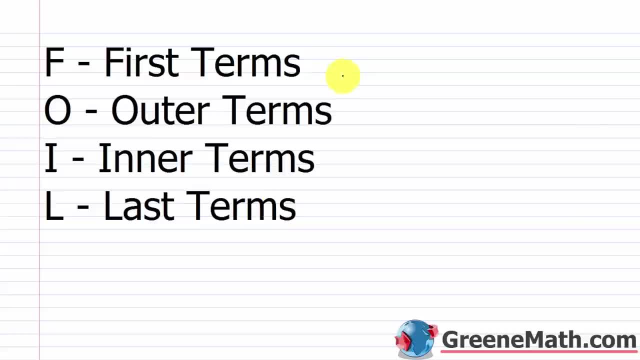 to multiply the final terms. So my third step is to multiply the final terms together. And then, when you first hear about FOIL, it seems a little confusing. You're like: well, what are the first terms, What are the outer terms? Once you do it, let's say 10 or 15 times, this becomes a method. 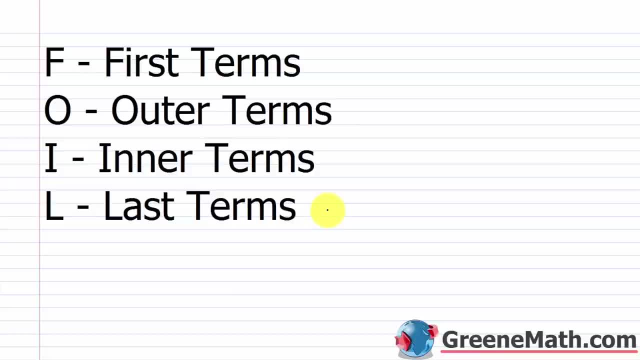 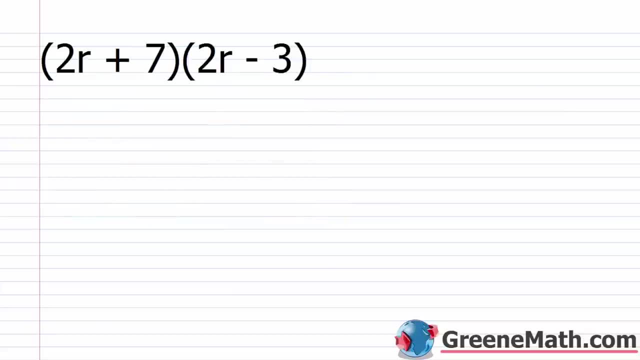 that you use for the rest of your life. I go through every time I multiply two binomials together. I use FOIL because it's just really, really easy to keep track of what's going on. So let's start out with this first problem, And the first way I'm going to do it is the way I showed you in the last. lesson. So I have 2r plus 7 times 2r minus 7.. And I'm going to do it in the same way I did in the last lesson. So I have 2r plus 7 times 2r minus 7.. And I'm going to do it in the same way I did in the 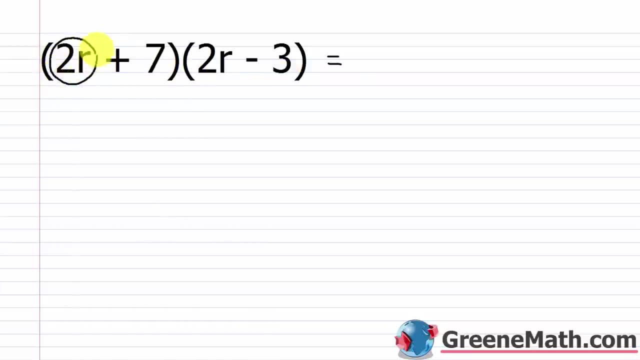 last lesson. So in the last lesson I kind of took each term from the first polynomial and just multiplied it by the second. So I did 2r times 2r minus 3.. And then plus, I would do 7 times 2r. 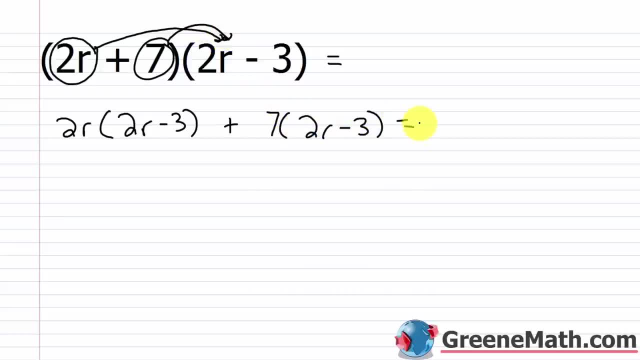 minus 3.. And this is not wrong, right? We can still use this. So 2r times 2r is 4r, squared. 2r times negative 3 is minus 6r And then plus 7 times 2r is 14r And then 7 times negative 3 is minus. 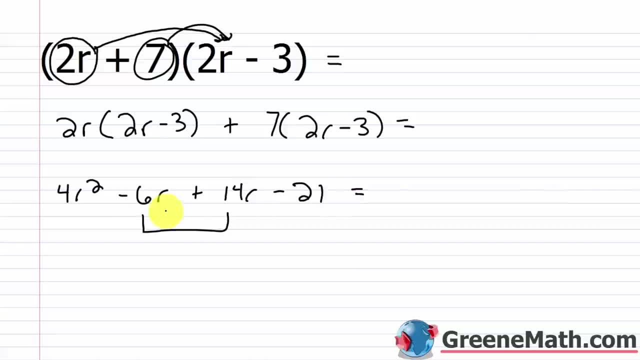 21.. So I would combine like terms here. We would have 4r squared And then negative. 6 plus 14 would be positive 8. So this would be plus 8r And then minus 21. So you get 4r squared plus 8r minus 21.. 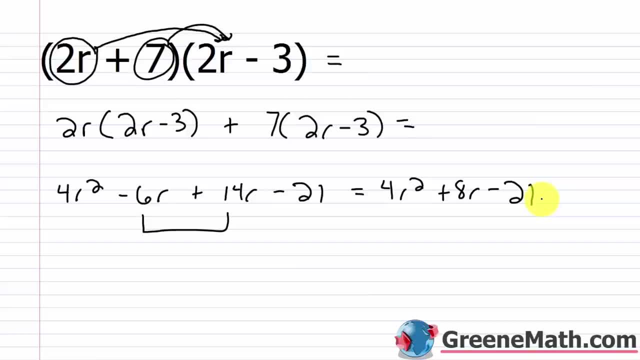 Now, if I had used FOIL, I would get the same thing, And let me kind of drag this answer up here, I'm going to erase everything else. If I used FOIL, f stands for first terms, So you multiply the first terms together, So this is the first one in this. 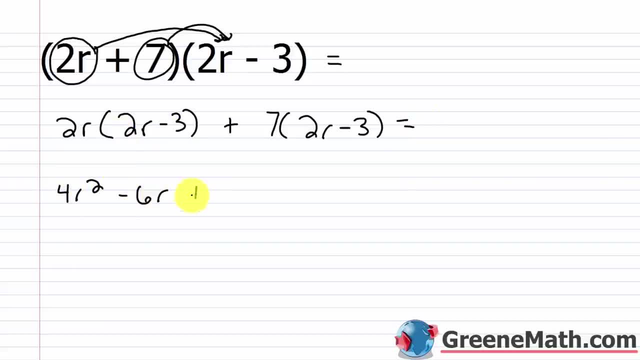 2r times negative 3 is minus 6r. And then plus, 7 times 2r is 14r. And then 7 times negative 3 is minus 21. So I would combine like terms here. We would have 4r squared. And then negative 6 plus 14 would be positive 8. So this would be plus 8r. And then minus 21. So you get 4r squared plus 8r minus 21. 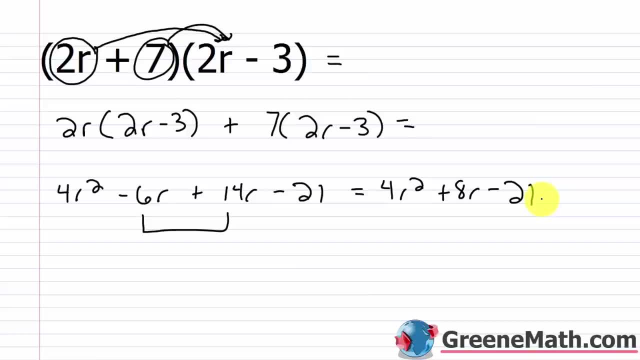 Now, if I had used FOIL, I would get the same thing. 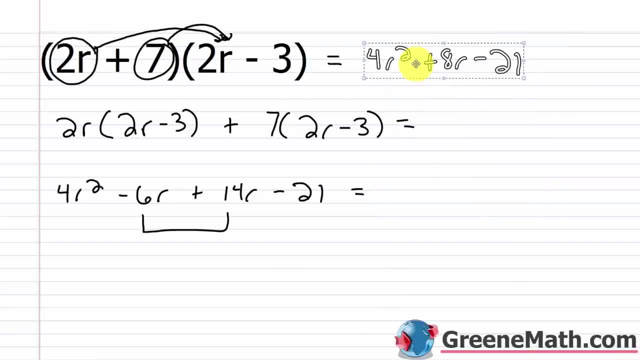 Let me kind of drag this answer up here. I'm going to erase everything else. If I used FOIL, F stands for first terms. So you multiply the first terms together. So this is the first one in this polynomial. This is the first one in this one. So 2r. So 2r times 2r is 4r squared. 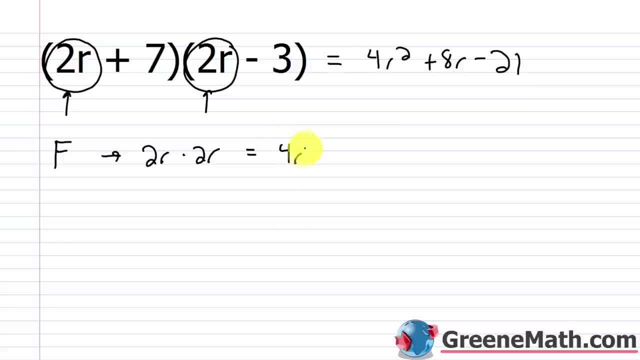 So 2r times 2r gives me 4r squared. 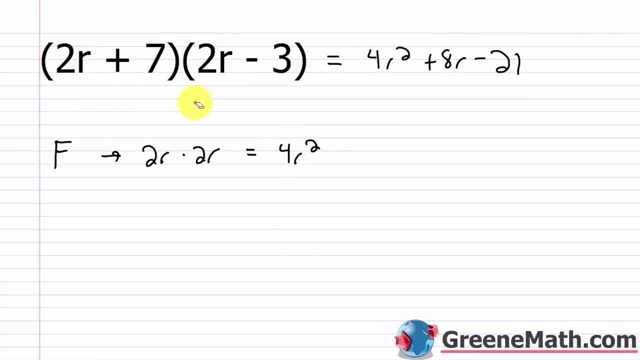 Then I would do my outer terms. My outer terms. So what's on the outside? This is on the outside. This is on the outside. 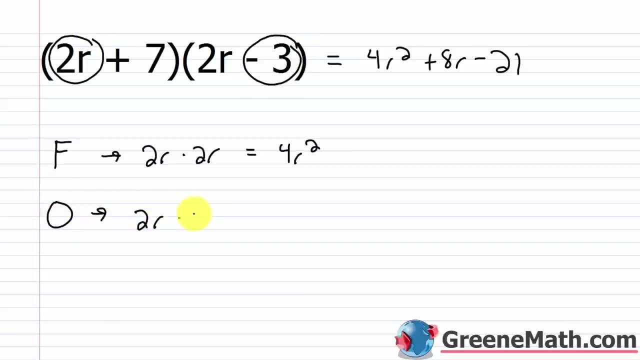 So for my outer terms, I'm going to do 2r times negative 3. So 2 times negative 3 is negative 6. Then times r, I get negative 6r. Then I would do my inner terms. 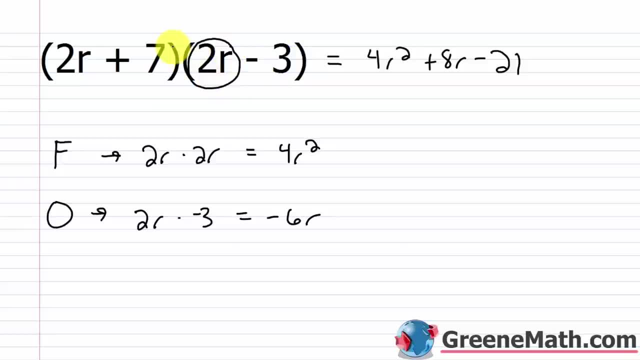 So what's on the inside? So this is on the inside. And this is on the inside. 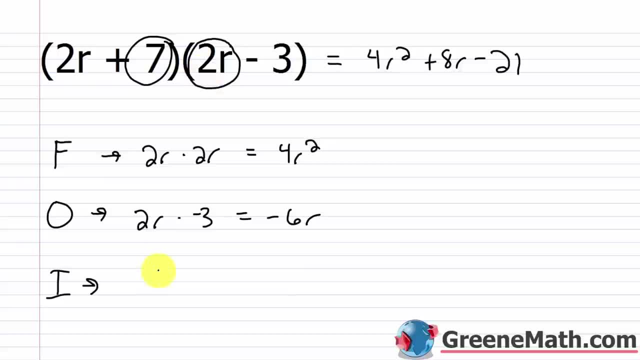 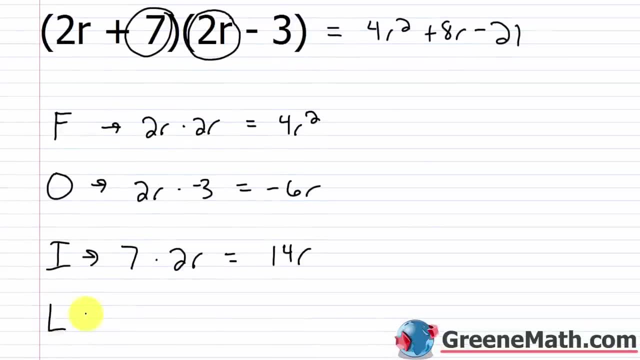 So I get my inner terms. I get 7 times 2r. 7 times 2r. That gives me 14r. And then lastly, I do my last terms. 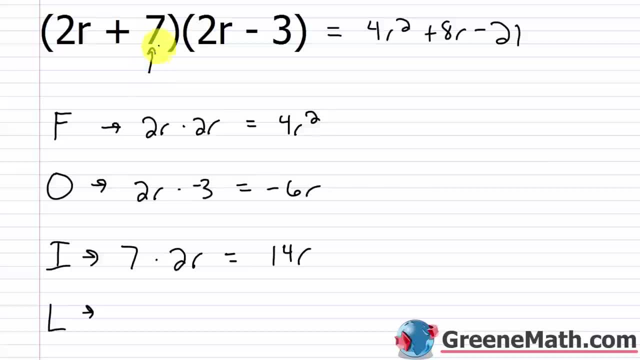 My l or my final terms. So this is the final term here. 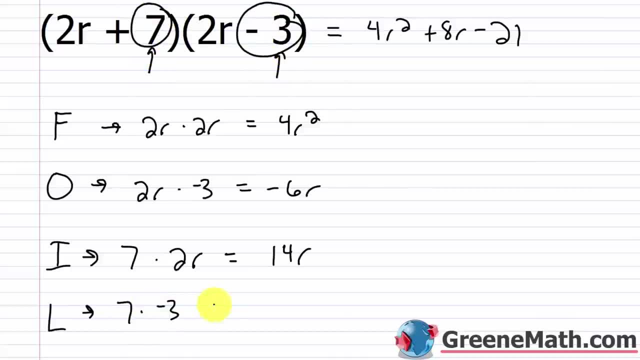 So I get 7 times negative 3. And that's negative 21. So I have 4r squared. I have negative 6r. I have 14r. And I have negative 21. 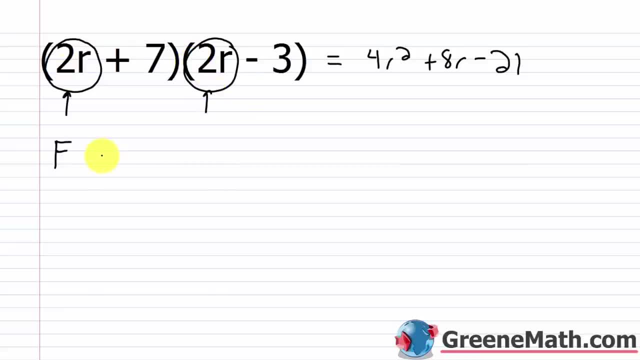 polynomial. This is the first one in this one. So 2r times 2r is 4r squared. So 2r times 2r gives me 4r squared. Then I would do my outer terms my outer terms. So what's on the outside? 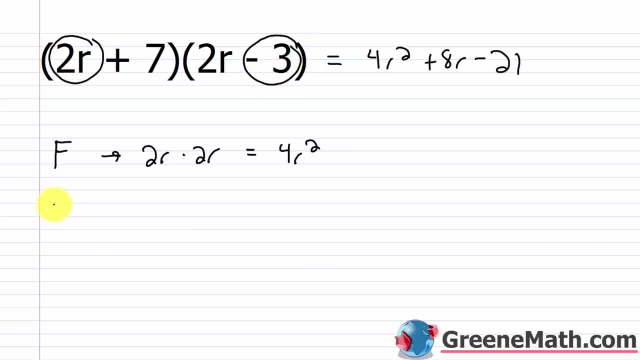 This is on the outside. This is on the outside. So for my outer terms I'm going to do 2r times negative 3.. So times negative three is negative six, Then times r, I get negative six r. Then I would do my inner. 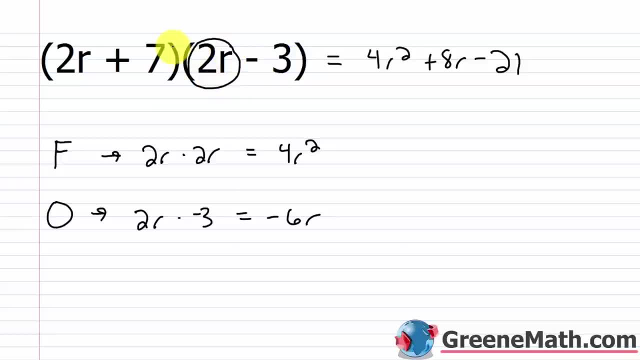 terms. So what's on the inside? So this is on the inside and this is on the inside. So I get my inner terms. I get seven times two r. seven times two r, That gives me 14r. And then, lastly, I do my. 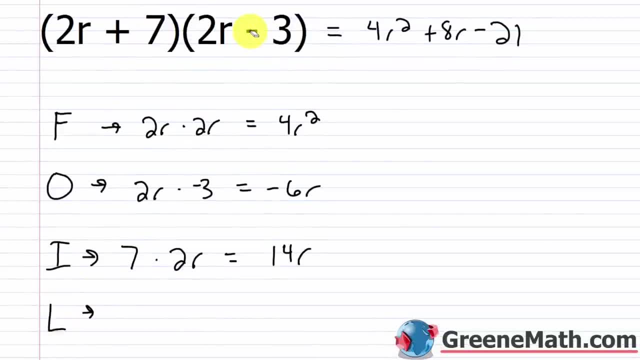 last terms, my l or my final terms. So this is the final term here. This is the final term here. So I get seven times negative three and that's negative 21.. So I have four r squared, I have negative six r, I have 14r and I have negative 21.. So if I combine like terms, you would see that 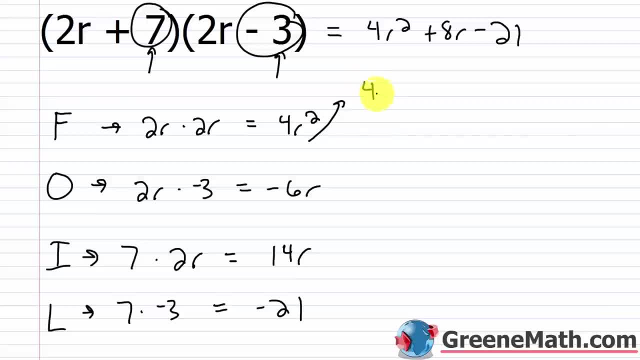 you get the exact same thing as you got here. You would end up with four r squared negative six r, plus 14r again would be plus eight r, And then you'd have minus 21.. So this FOIL method is not. 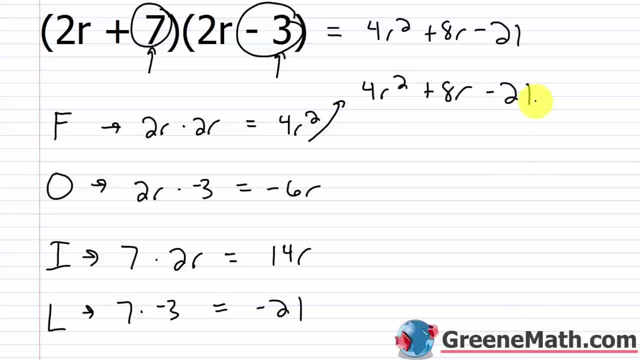 producing a different result. It's producing a different result. It's producing a different. so this FOIL method is not producing a different result. It's producing a different result. It's result. It's just a convenient way to remember how to get the product of two binomials. And again, 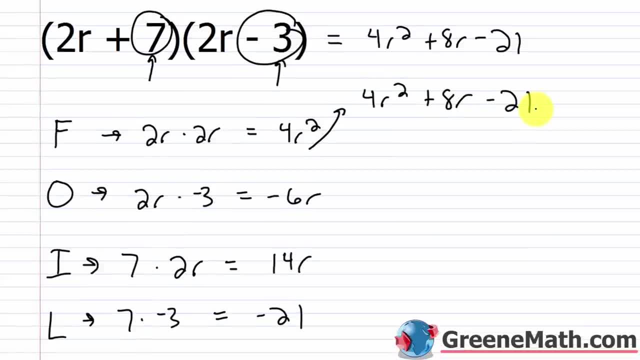 once you start using this, you're going to love it, Something you're going to use for the rest of your life. All right, let's take a look at this one. We have 5n plus 5 times 6n minus 2.. 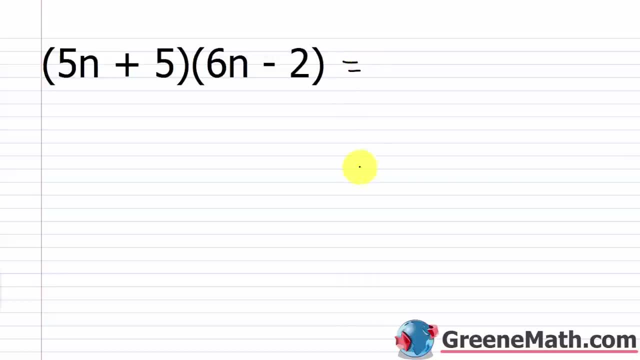 So let's use FOIL. So I want to start out with the F first terms. So the first terms we have: 5n times 6n. 5 times 6 is 30.. n times n is n squared. Now I want to use my outer terms. 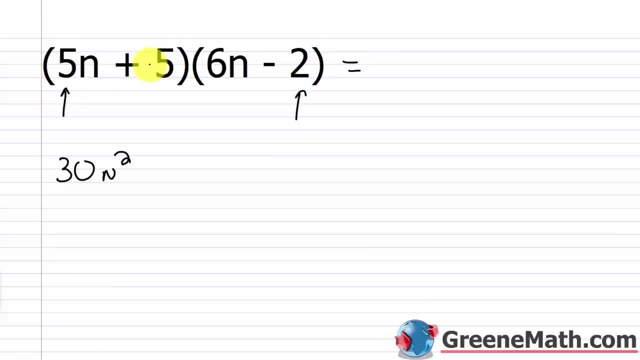 So here's the outer term. Here's the outer term. So my outside terms: 5n times negative 2 would be negative 10n. Now I want to do my inner terms. So I want to do 5 times 6n. So these are: 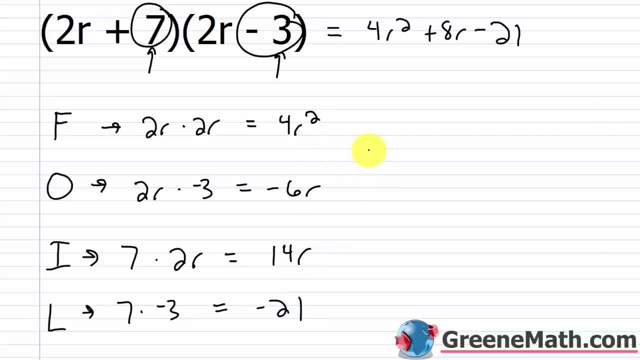 So if I combine like terms, you would see that you get the exact same thing as you got here. You would end up with 4r squared. Negative 6r plus 14r, again, would be plus 8r. And then you'd have minus 21. So this FOIL method is not producing a different result. It's just a convenient way to remember how to get the product of two binomials. And again, once you start using this, you're going to love it. It's something you're going to use for the rest of your life. All right, let's take a look at this one. 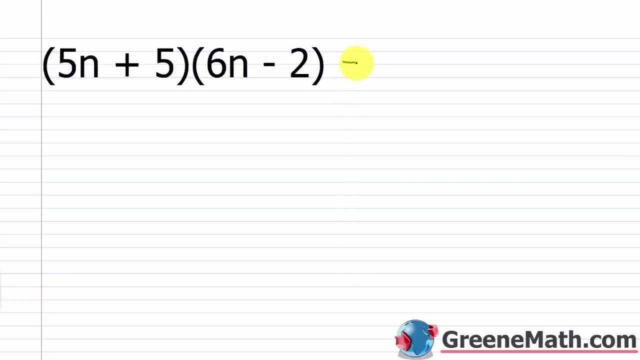 We have 5n plus 5 times 6n minus 2. So let's use FOIL. So I want to start out with the f, first terms. So the first terms, we have 5n times 6n. 5 times 6 is 30. n times n is n squared. Now I want to use my outer terms. So here's the outer term. Here's the outer term. So my outside terms. 5n times negative 2 would be negative 10n. 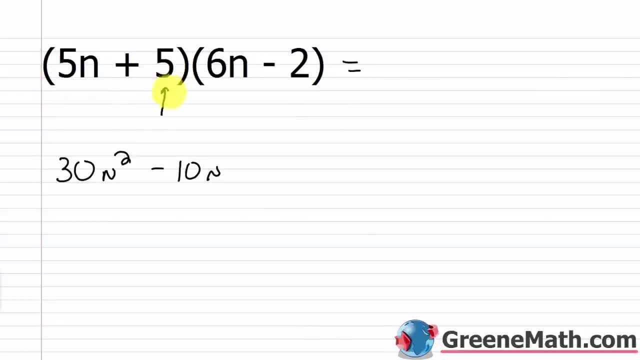 Now I want to do my inner terms. So I want to do 5 times 6n. So these are on the inside. 5 times 6 is 30. Then times n. So 30n. Then I want to do my last or final terms. 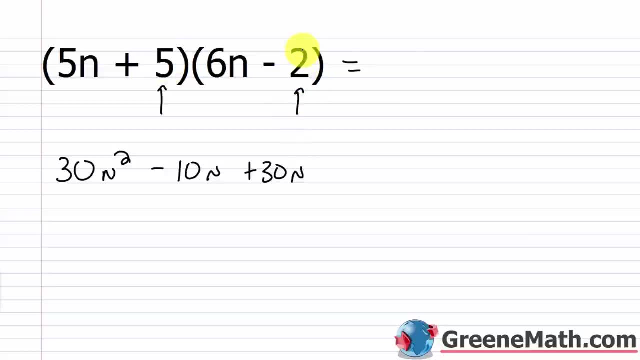 So I got 5 here as the final term. Negative 2 here is the final term. 5 times negative 2 is negative 10. And so I've got 30n squared minus 10n plus 30n minus 10. 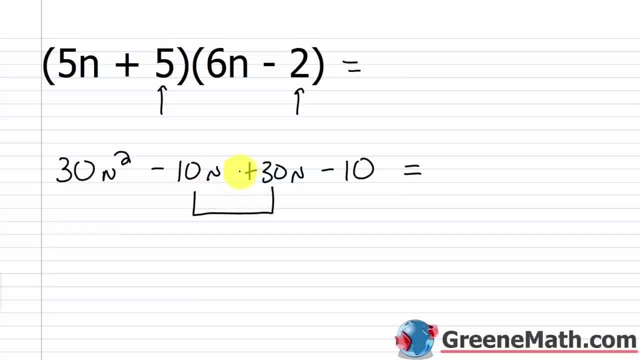 So all I need to do now is just combine like terms here. Negative 10n plus 30n is 20n. So this gives me a final answer of 30n squared plus 20n minus 10. All right. 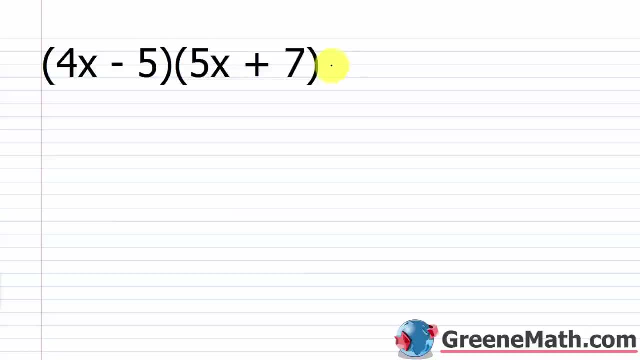 For the next one, I have 4x minus 5 times 5x plus 7. 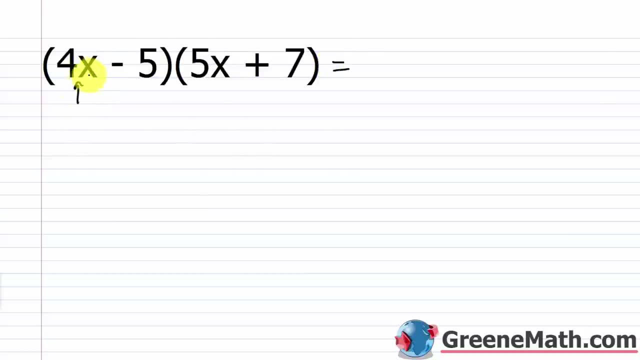 So again, I'm going to use FOIL. So first terms, I have 4x and I have 5x. 4x times 5x is 20x squared. Then I'm going to move to the outer terms, the o. So that's 4x times 7. 4x times 7 is 28x. So plus 28x. Then I'm going to move to my inside terms. So I have negative 5 and I have 5x. 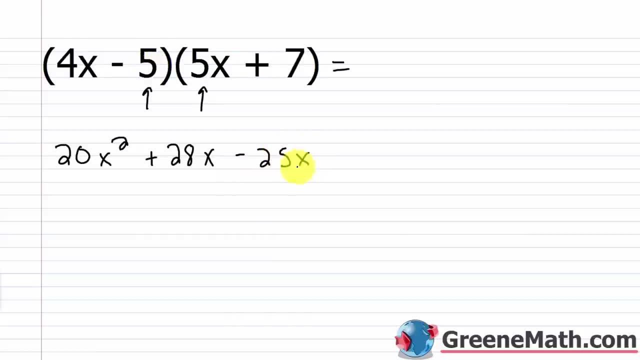 So negative 5 times 5x is negative 25x. 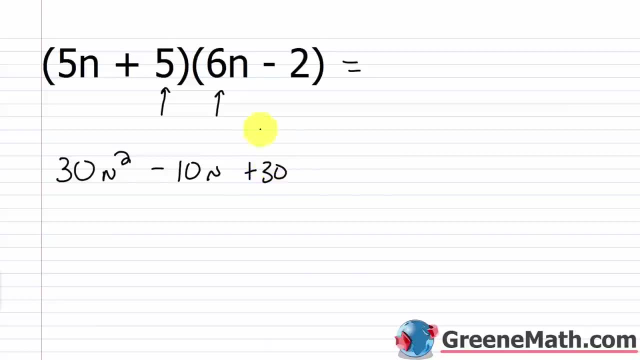 the inside: 5 times 6 is 30. Then times n, So 30n. Then I want to do my last or final terms. So I got 5- here is the final term. Negative 2: here is the final term. 5 times negative, 2 is negative 10.. 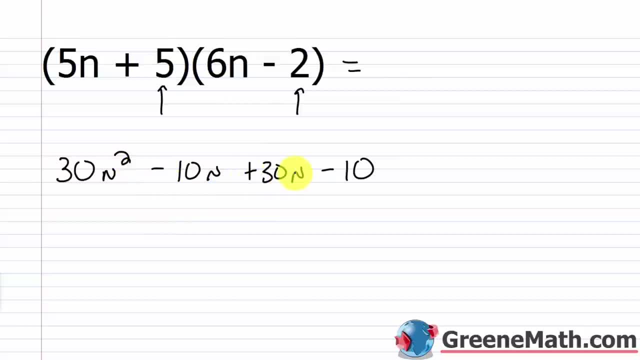 And so I've got 30n squared minus 10n plus 30n minus 10.. So all I need to do now is just combine like terms here: Negative 10n plus 30n is 20n, So this gives me a final answer of 30n squared. 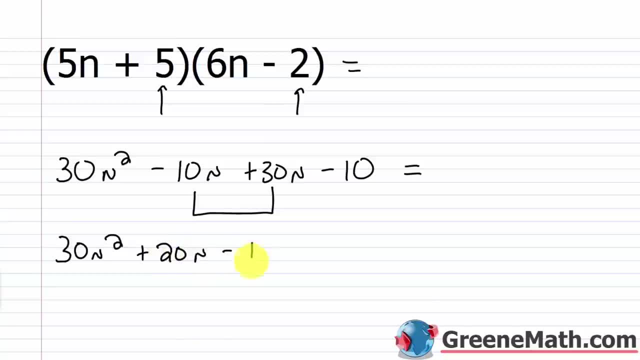 plus 20n minus 10.. All right, for the next one. I have 4x minus 5 times 5x plus 7.. So again, I'm going to use FOIL. So, first terms: I have 4x and I have 5x, 4x times 5x. 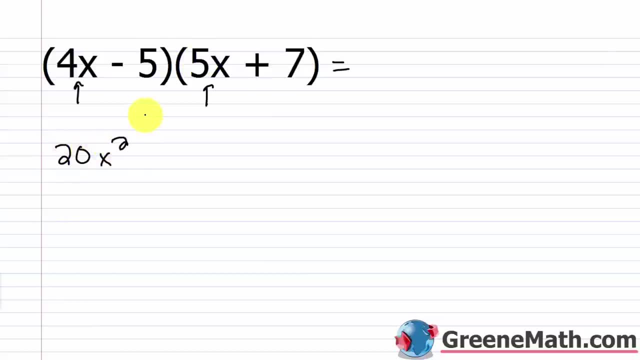 is 20x squared. Then I'm going to move to the outer terms, the O. So that's 4x times 7.. 4x times 7 is 28x. So plus 28x. Then I'm going to move to my inside terms. So I have negative 5 and I have 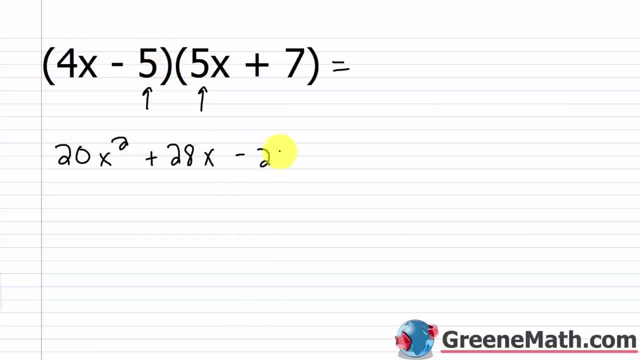 5x. So negative 5 times 5x is negative 25x. Then I'm going to move to my last or final terms, So 5 times 7.. And that's going to give me negative 35.. So all I need to do now is just combine like: 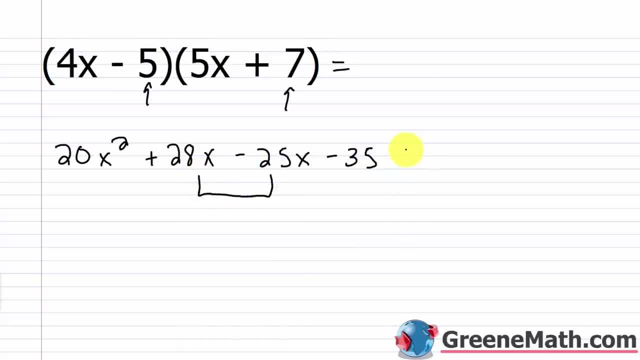 terms, I have 28x minus 25x. That's going to give me 3x. So this would be 20x squared plus 3x minus 35 as my final answer. All right, what about 7x minus 7 times 4x plus 2?? Again, I'm going to use 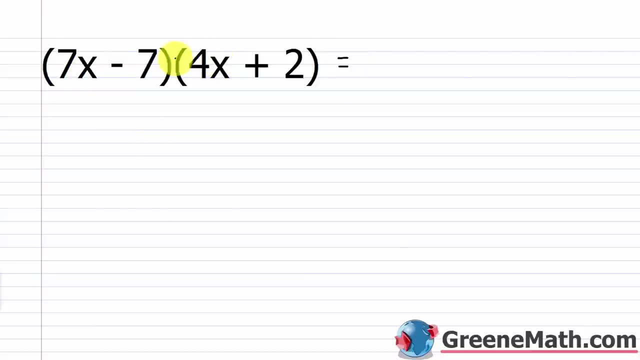 FOIL. So my first terms: I have 7x and I have 4x. 7x times 4x is 28x squared. My outer terms: 7x times 2, would be plus 14x. My inside terms: I have negative 7. 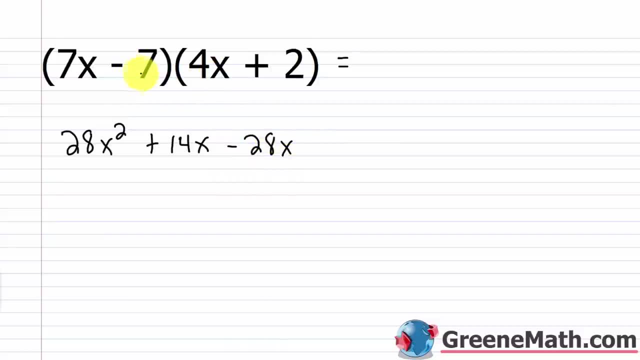 times 4x, That's negative 28x. And then my last terms, I have negative 7 times 2. That's negative 14.. So we end up with 28x squared 14x. minus 28x is negative 14x And then minus 14.. 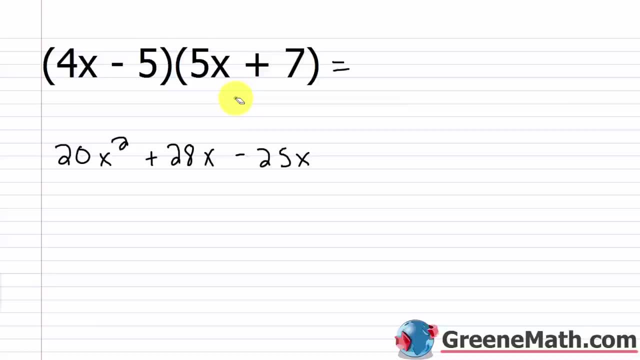 Then I'm going to move to my last or final terms. So that's negative 5 times 7. And that's going to give me negative 35. 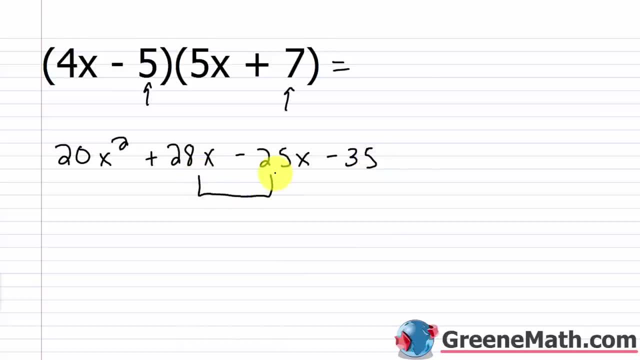 So all I need to do now is just combine like terms. I have 28x minus 25x. That's going to give me 3x. 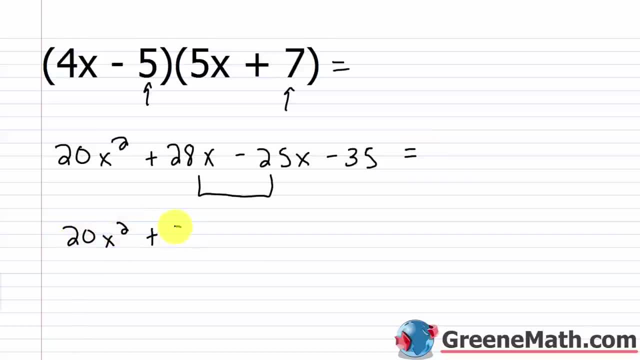 So this would be 20x squared plus 3x minus 35 as my final answer. All right. 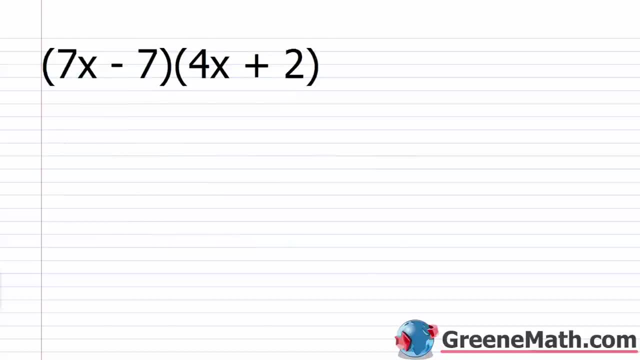 What about 7x minus 7 times 4x plus 2? Again, I'm going to use FOIL. So my first terms, I have 7x and I have 4x. 7x times 4x is 28x squared. My outer terms, 7x times 2, would be plus 14x. My inside terms, I have negative 7 times 4x. That's negative 28x. And then my last terms, I have negative 7 times 2. 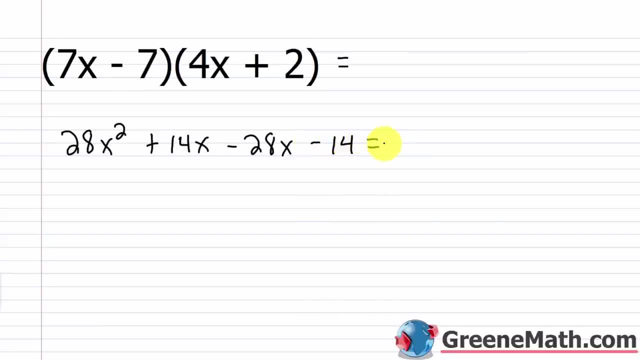 That's negative 14. So we end up with 28x squared. 14x minus 28x is negative 14x. And then minus 14. So 28x squared minus 14x minus 14 is my answer. All right. Let's take a look at another one. 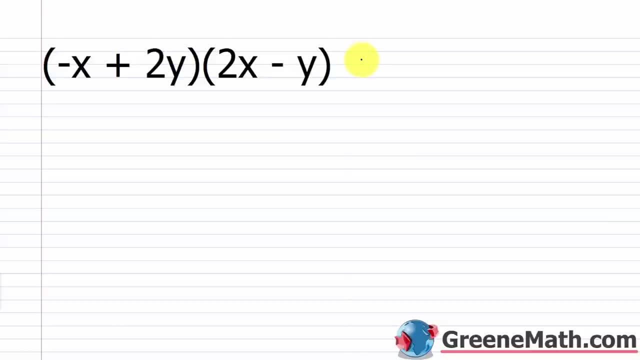 I have negative x plus 2y times 2x minus y. So I'm going to do my first terms. 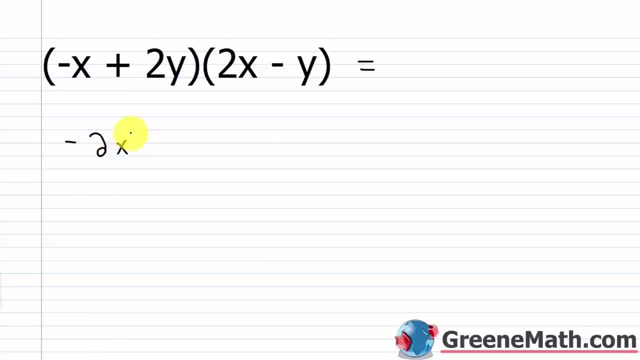 Negative x times 2x is negative 2x squared. I'm going to do my outer terms. 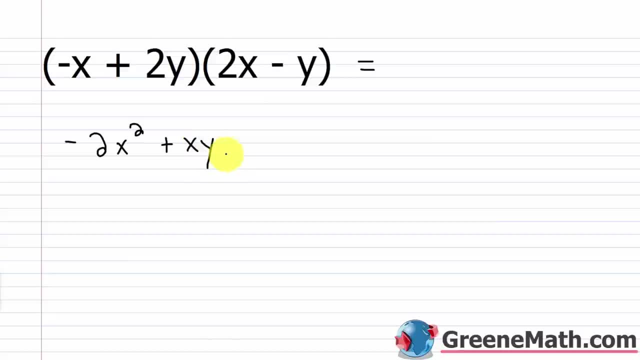 Negative x times negative y is plus xy. I'm going to do my inside terms. 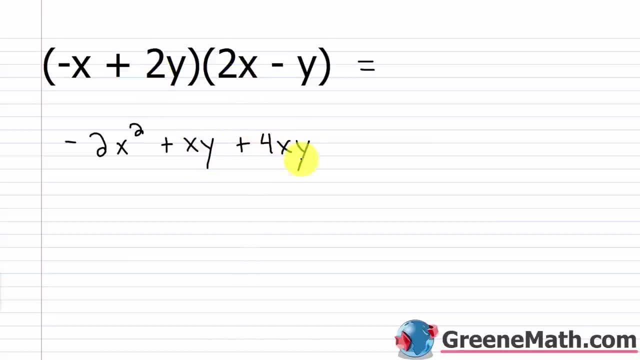 2y times 2x would be plus 4xy. And then I'm going to do my last terms. 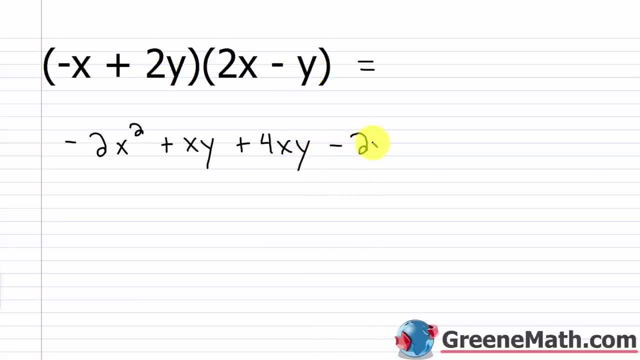 2y times negative y is going to be negative 2y squared. 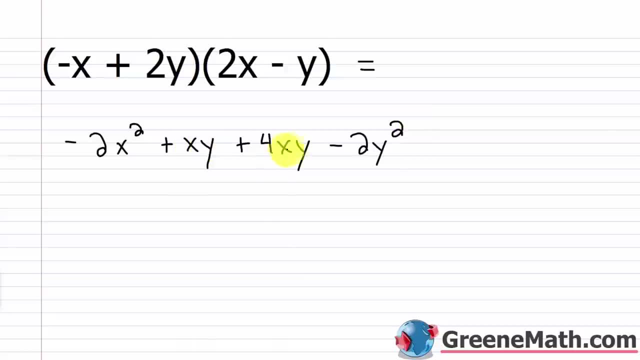 So what can I do here to combine like terms? I have xy and I have 4xy. 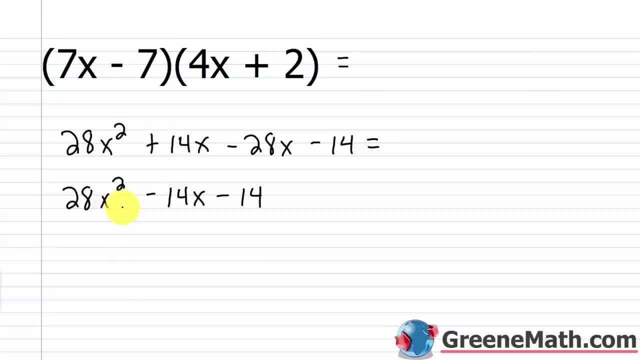 So 28x squared minus 14x minus 14 is my answer. All right, let's take a look at another one. I have negative x plus 2y times 2x minus y. So I'm going to do my first terms: Negative x times 2x. 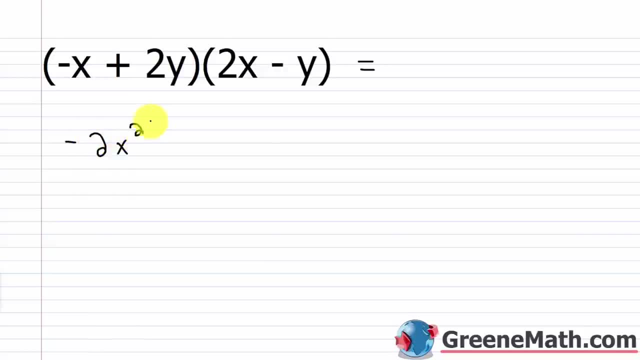 is negative 2x squared. I'm going to do my outer terms: Negative x times negative y is plus xy. I'm going to do my inside terms: 2y times 2x would be plus 4xy. And then I'm going to do my last. 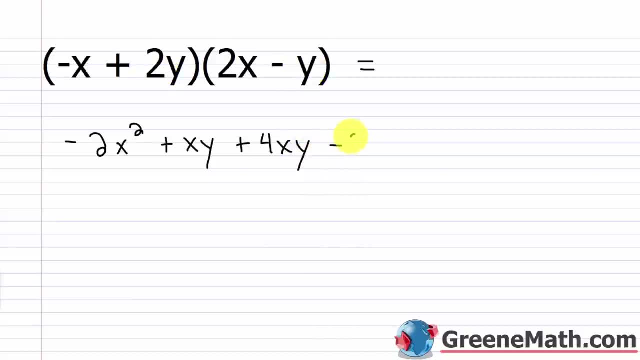 terms: 2y times negative, y is going to be negative 2y squared. So what can I do here to combine like terms? I have xy and I have 4xy, So those are like terms. So basically you think of: 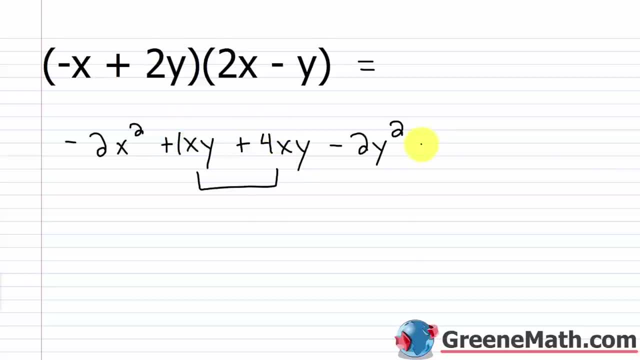 this again as 1xy plus 4xy. 1 plus 4 is 5.. So this ends up being negative 2x squared plus this would be 5xy, and then minus 2y squared. Let me kind of make this a little better. 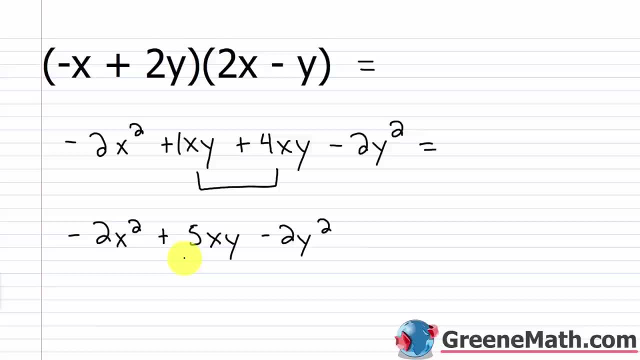 Again, our answer is negative: 2x squared plus 5xy minus 2y squared. All right, let's take a look at negative: 5x minus 3y times 2x plus 4y. So my first terms: negative 5x times 2x. Negative 5. 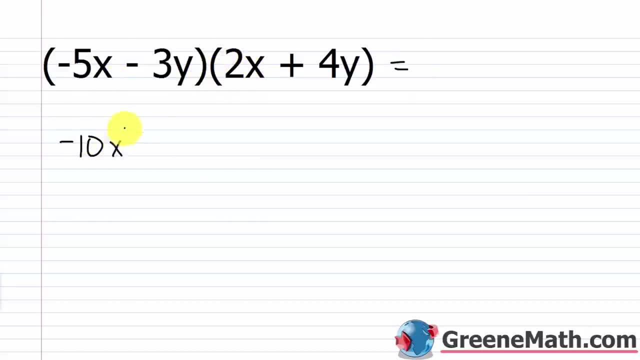 times 2 is negative 10.. x times x is x squared. My outer terms: negative: 5x times 4y, That's negative 20xy. My inner terms: negative: 3y times 2x, That's negative 6xy. 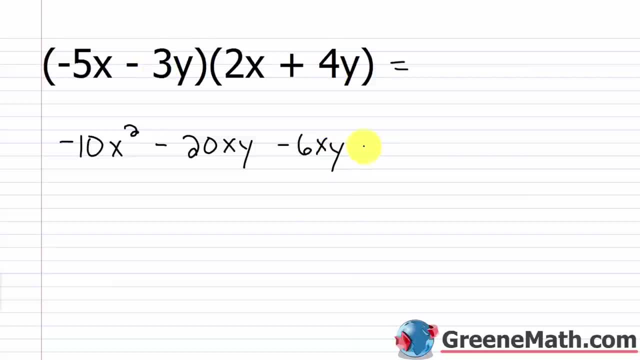 And then my last or final terms: negative 3y times 4y is negative 12y squared. So here are my like terms in the middle here: Negative 20 minus 6 would be negative 26. So you get negative 26xy. 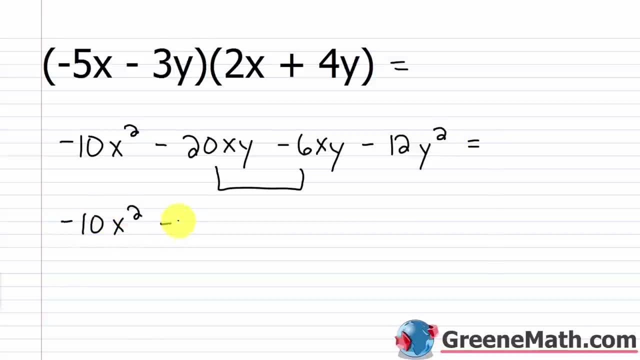 So you'd have negative 10x squared and then minus 26xy and then minus 12y squared. So again my answer: negative 10x squared minus 26xy, minus 12y squared. All right. for the next one, we have 3x plus 5y times negative 8x minus 7y. 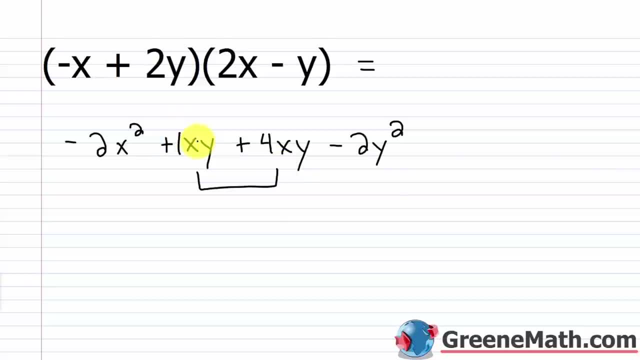 So those are like terms. So basically you think of this again as 1xy plus 4xy. 1 plus 4 is 5. So this ends up being negative 2x squared plus this would be 5xy and then minus 2y squared. 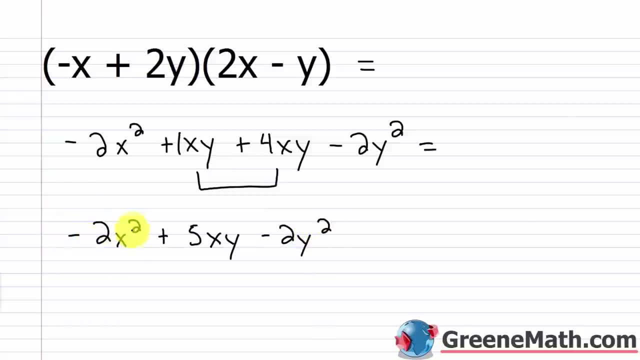 Let me kind of make this a little better. Again, our answer is negative 2x squared plus 5xy minus 2y squared. 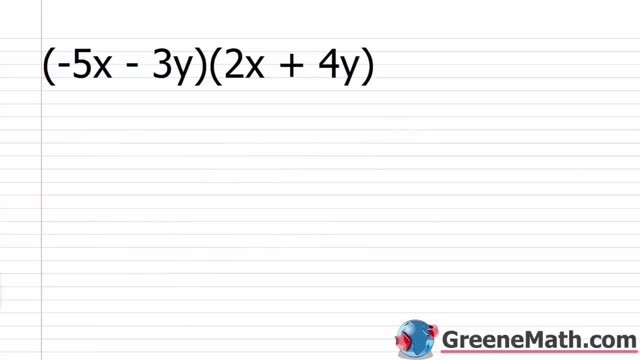 Now let's take a look at negative 5x minus 3y times 2x plus 4y. 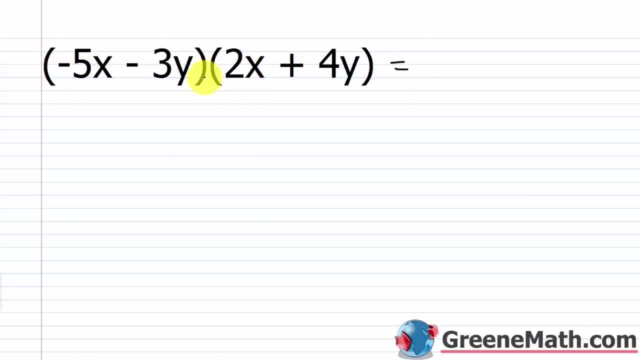 So my first terms. Negative 5x times 2x. Negative 5 times 2 is negative 10. 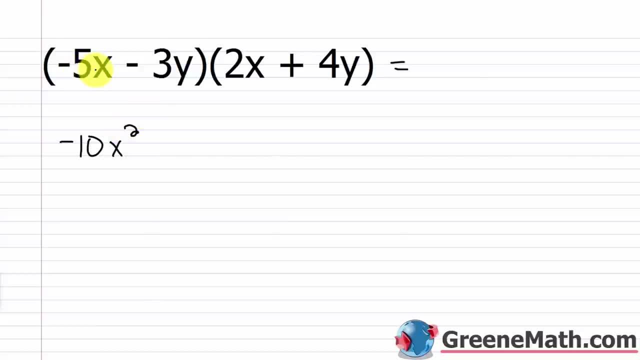 x times x is x squared. My outer terms. Negative 5x times 4y. That's negative 20xy. 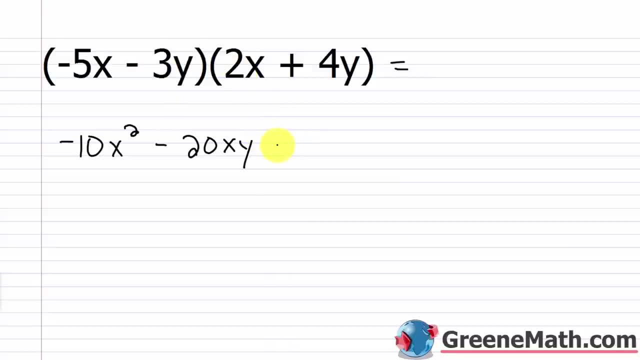 My inner terms. Negative 3y times 2x. That's negative 6xy. 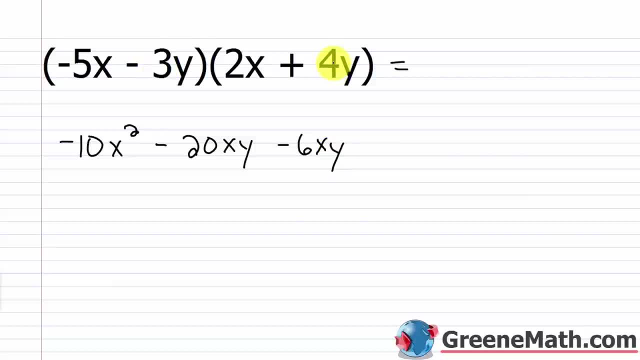 And then my last or final terms. Negative 3y times 4y is negative 12y squared. So here are my like terms in the middle here. 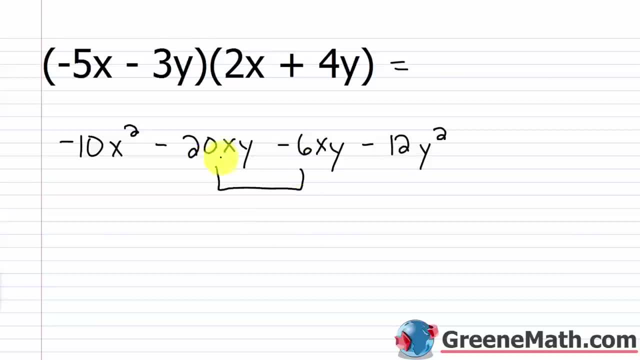 Negative 20 minus 6 would be negative 26. So you get negative 26xy. 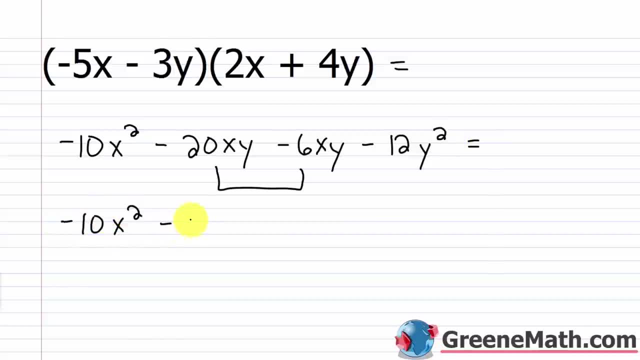 So you'd have negative 10x squared and then minus 26xy and then minus 12y squared. 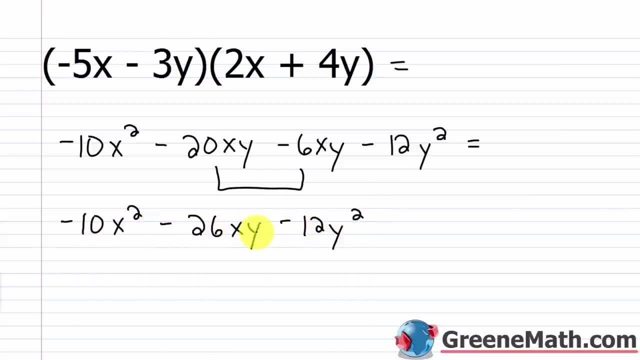 So again, my answer is negative 10x squared minus 26xy minus 12y squared. 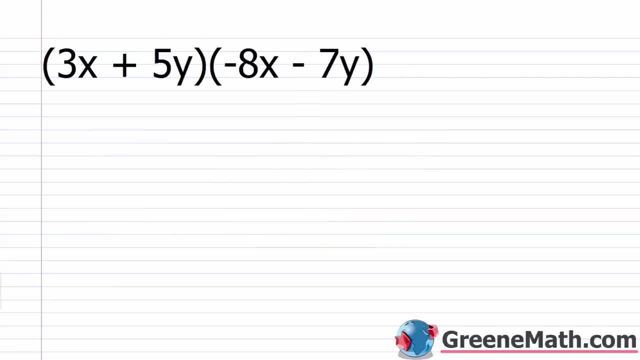 Alright, for the next one we have 3x plus 5y times negative 8x minus 7y. So 3x times negative 8x is negative 24x squared. Then 3x times negative 7y is minus 21xy. Then 5y times negative 8x is minus 40xy. Then 5y times negative 7y is minus 35y squared. Alright, so now we want to combine the like terms in the middle here. 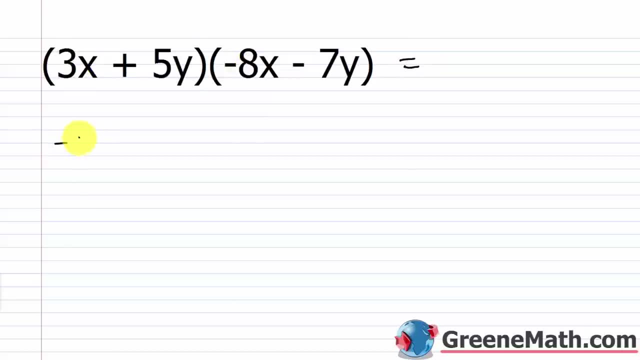 So 3x times negative, 8x is negative 24x squared. Then 3x times negative, 7y is minus 21xy. Then 5y times negative, 8x is minus 40xy. Then 5y times negative 7y is minus 35y squared. 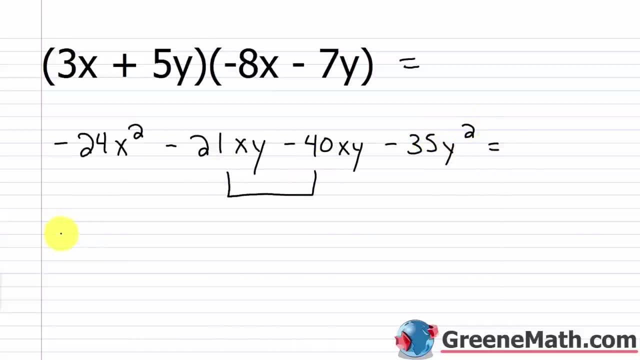 All right. so now we want to combine the like terms in the middle here. So I'd have negative 24x squared- I'm going to make that a little better- And then negative 21xy minus 40xy would be negative 61xy, And then we have minus 35y squared. So again, the answer here would be: 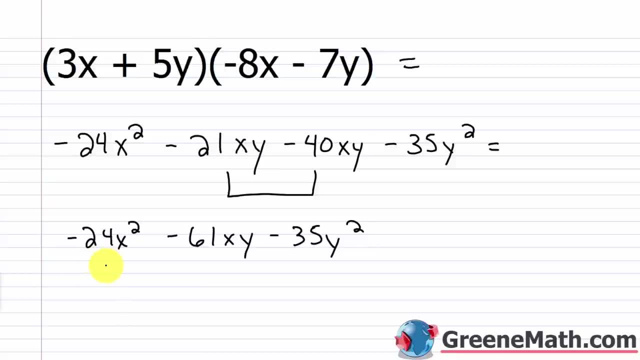 negative 24x squared minus 61xy, minus 35y squared. All right, so for this last problem here we can't use FOIL to get the product of three binomials. But what we can do is we can use FOIL. 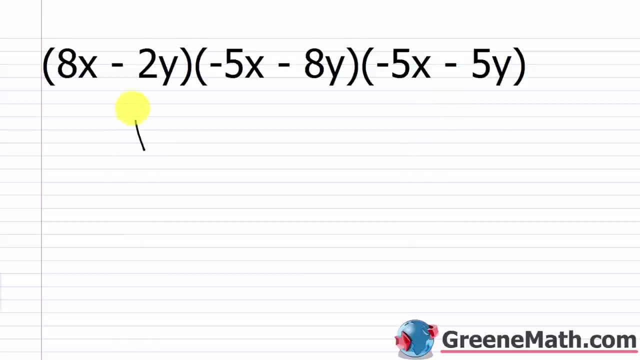 for the product of any two. So if I wanted to start out by multiplying these two together, I could use FOIL here. Then once I got that product, I can multiply this guy, whatever that product is by this guy. Again, you can only use FOIL for the product of two binomials. 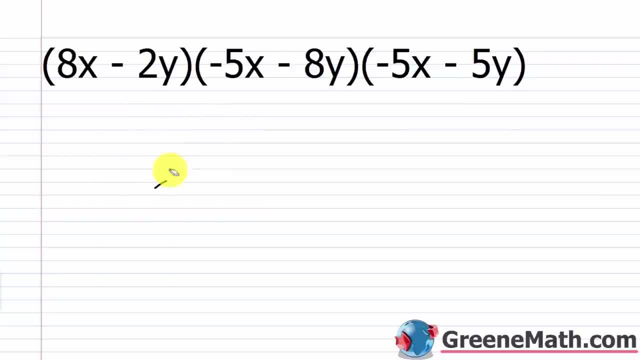 Very important that you understand that. So let's go ahead and use FOIL for the product of two binomials. Let's use FOIL to multiply these two together. So 8x times negative 5x. that would be my first terms. 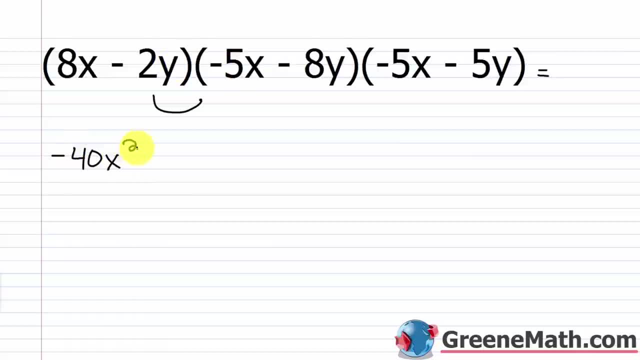 And that would give me negative 40x squared. My outside terms: 8x times negative 8y would be minus 64xy. My inside terms here: negative 2y times negative 5x would be plus 10xy. 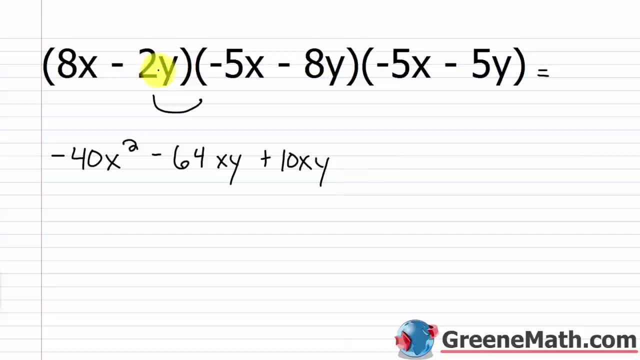 Then my last or final terms would be negative 2y times negative 8y, which would be plus 10xy. And then my outside terms, 8x times negative 8y, would be minus 64xy Plus 16y squared. Now that I have this, I want to combine like terms in the middle. 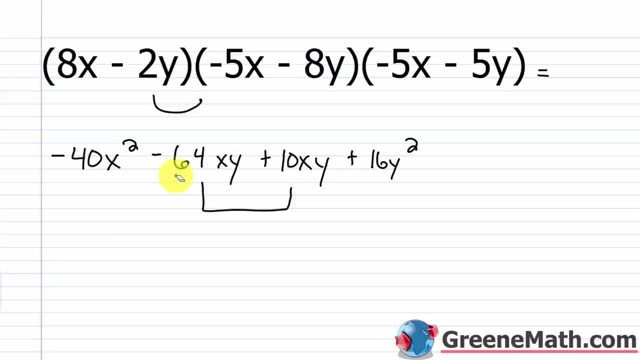 Negative 64xy plus 10xy is going to be negative 54xy. So I have this guy now, which is the result of the multiplication of these two binomials, and then times this guy. So I can't use FOIL here, because I have a binomial times a trinomial. 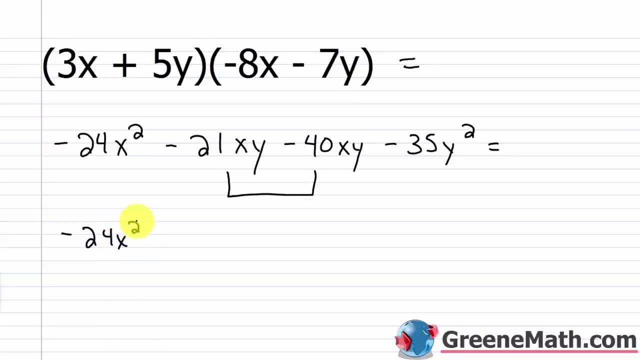 So I'd have negative 24x squared. Gonna make that a little better. And then negative 21xy minus 40xy would be negative 61xy. And then we have minus 35y squared. So again, the answer here would be negative 24x squared minus 61xy minus 35y squared. 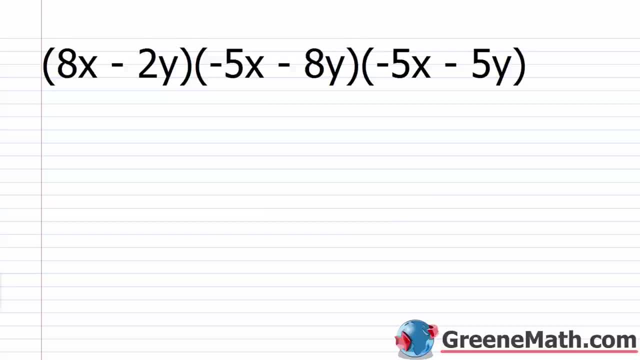 Alright, so for this last problem here, we can't use FOIL. We can use FOIL to get the product of three binomials. 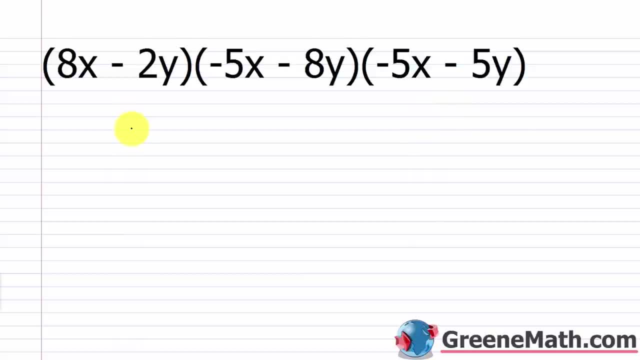 But what we can do is we can use FOIL for the product of any two. So if I wanted to start out by multiplying these two together, I could use FOIL here. Then once I got that product, I could multiply this guy, whatever that product is, by this guy. Again, you can only use FOIL for the product of two binomials. Very important that you understand that. 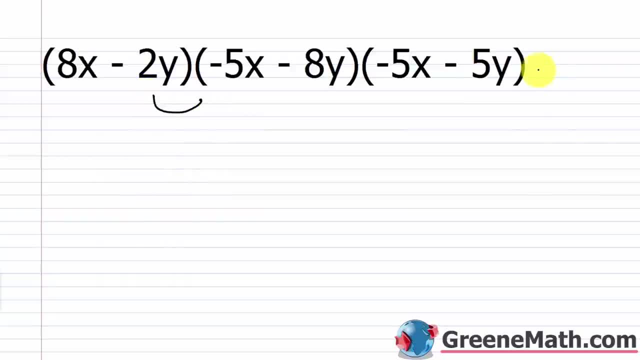 So let's go ahead and use FOIL to multiply these two together. So 8x times negative 5x, that would be my first terms. And that would give me negative 40x squared. My outside terms, 8x times negative 8y, would be minus 64xy. 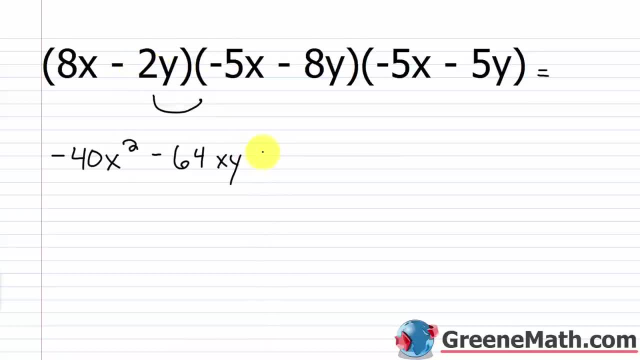 My inside terms here, negative 2y times negative 5x, would be plus 10xy. 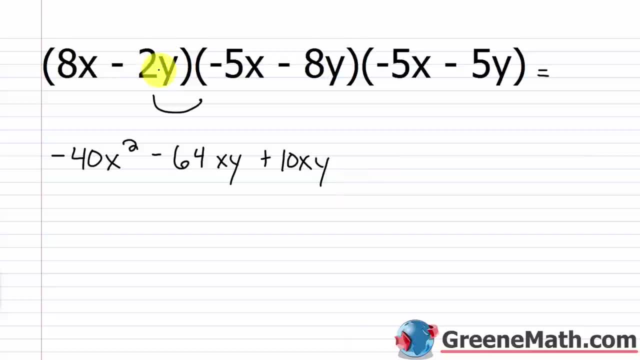 Then my last or final terms, would be negative 2y times negative 8y, which would be plus 16y. 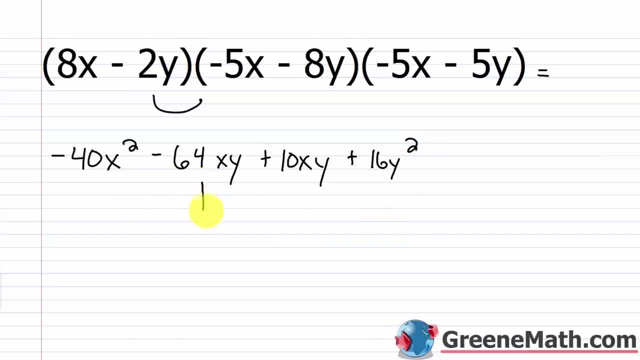 Now that I have this, I want to combine like terms in the middle. 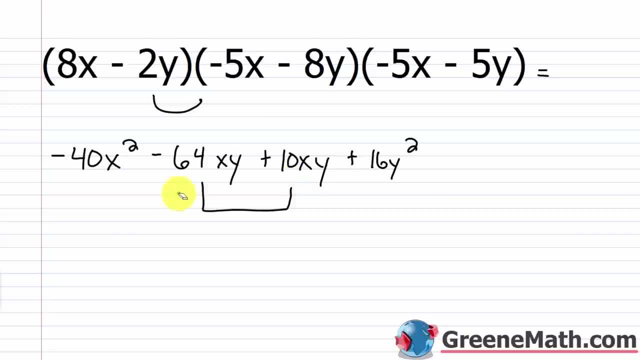 Negative 64xy plus 10xy is going to be negative 54xy. 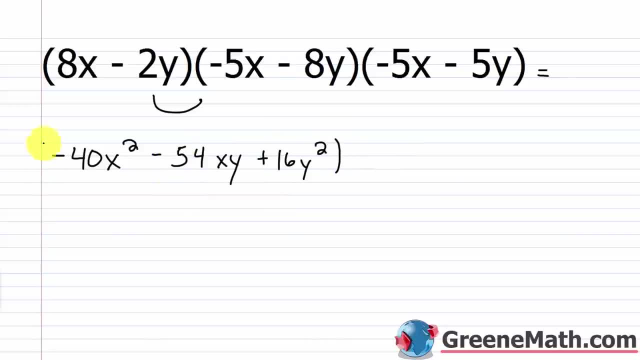 So I have this guy now, which is the result of the multiplication of these two binomials, and then times this guy. So I can't use FOIL here, because I have a binomial times a trinomial. FOIL does not work. Please don't try that. You've got to use the original method that we talked about. 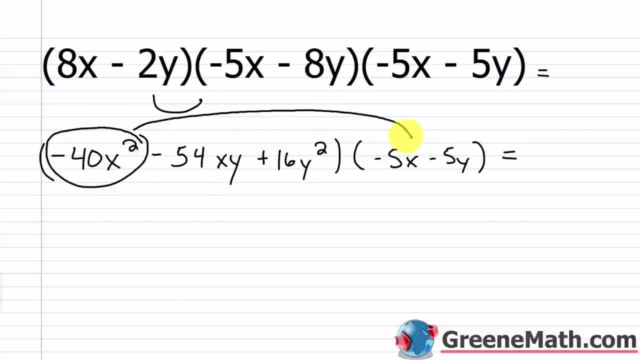 So you're going to take each term of this and multiply it by each term of this. 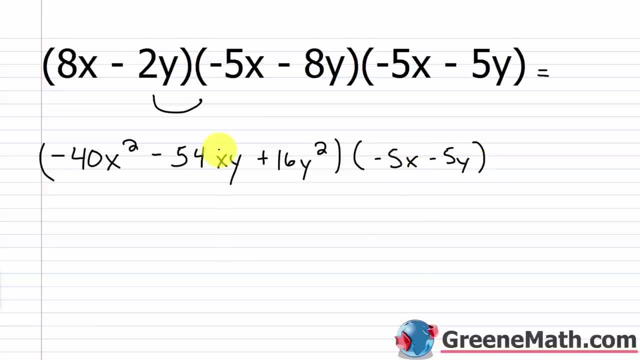 FOIL does not work. Please don't try that. You've got to use the original. So you're going to take each term of this and multiply it by each term of this. So I'll do negative 40x squared times negative 5x. That's going to be 200x cubed. 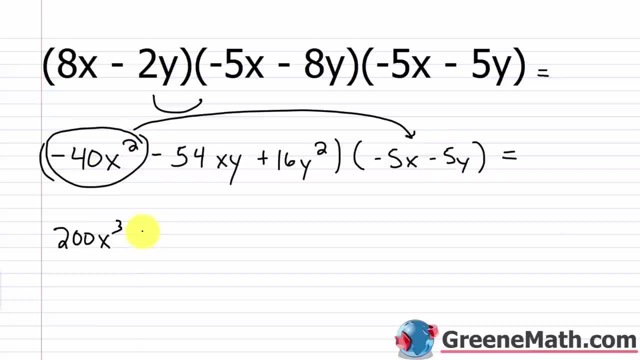 Then negative 40x squared times negative 5y, That's going to be plus 200x squared y. Then we'll go here. So negative 54xy times negative 5x, That's going to be positive 270x squared y. Then negative 54xy times negative 5y, That's going to be again. 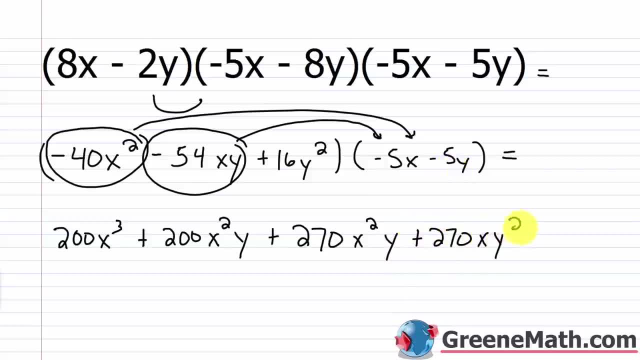 positive 270xy squared. Now I'm going to take this guy and multiply it by this polynomial. So 16y squared times negative 5x. 16 times negative 5 is negative 80. So that's negative 80. And then xy squared. And then 16y squared times negative 5x. 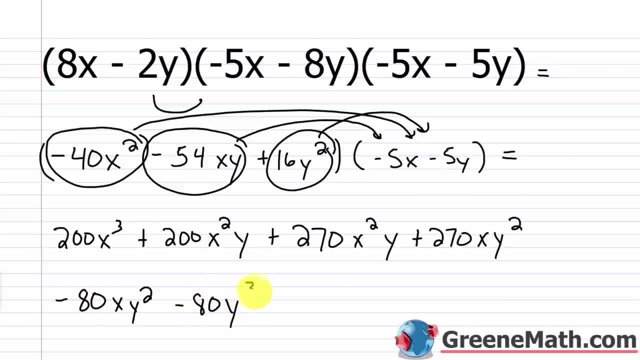 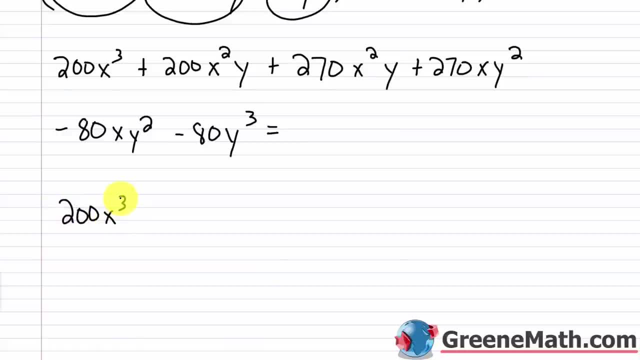 16y squared times negative 5y, That's negative 80y cubed. All right, Then this equals So 200x cubed. And then let's take a look at this: We have x squared y, x squared y. 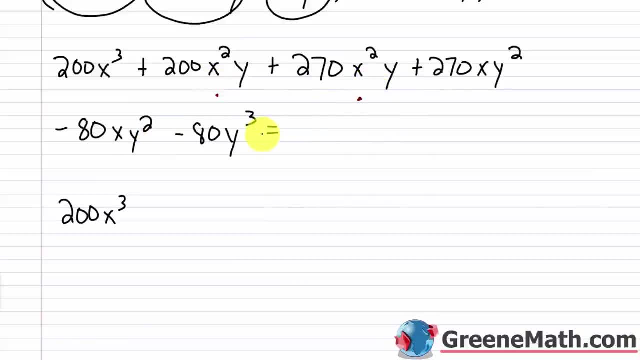 So no other like terms. Remember, for you to have like terms, it's got to be the same variable raised to the same power. So I've got to have an x squared and then a y to the first power. So that occurs here and here, Doesn't occur here, Doesn't occur here. 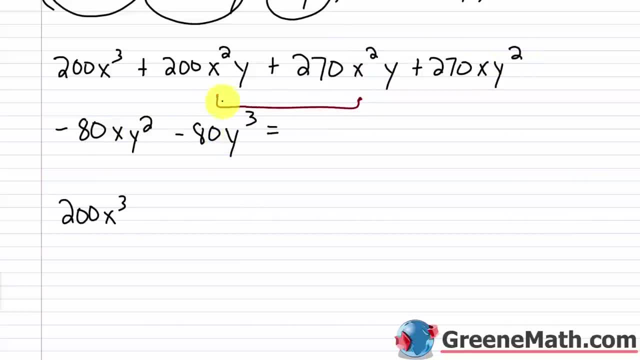 Or here. So just these two are like terms. So 200 plus 270 is 470.. And then x squared y, Now I have 270xy squared and negative 80xy squared. So these are like terms. These, and only these, can be combined together. So 270 minus 80 is 190.. So this would be plus. 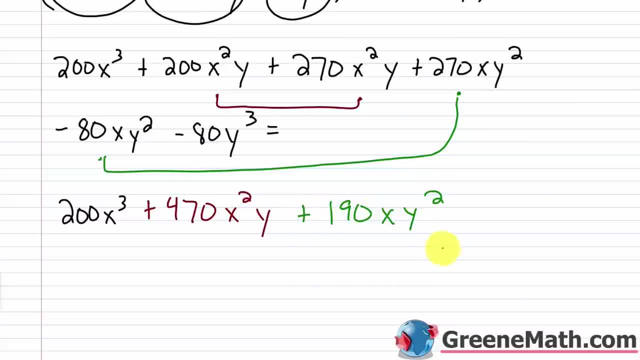 190xy squared. Lastly, I have minus 80y cubed. Nothing I can combine with that. So my answer here is 200x cubed plus 470x squared y plus 190xy squared minus 80y cubed. 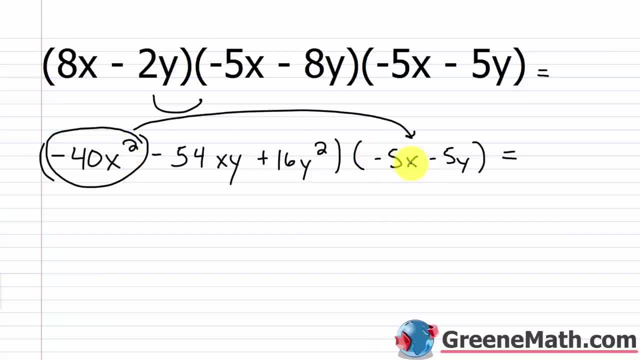 So I'll do negative 40x squared times negative 5x. That's going to be 200x cubed. Then negative 40x squared times negative 5y. That's going to be plus 200x squared y. Then we'll go here. 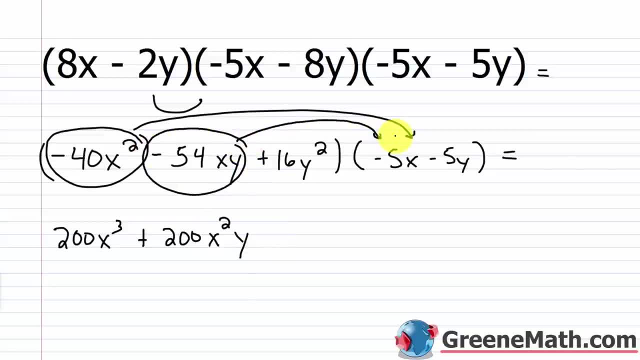 So negative 54xy times negative 5x. That's going to be positive 200x. 270x squared y. Then negative 54xy times negative 5y. 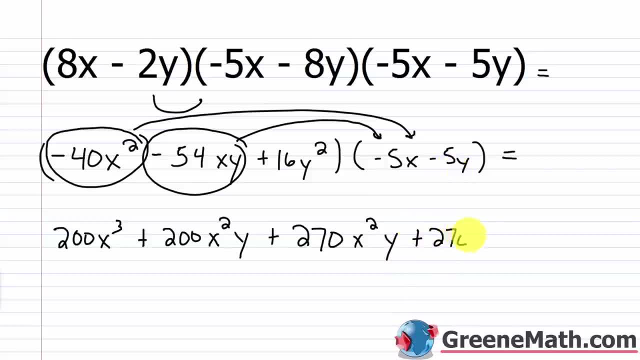 That's going to be, again, positive 270xy squared. 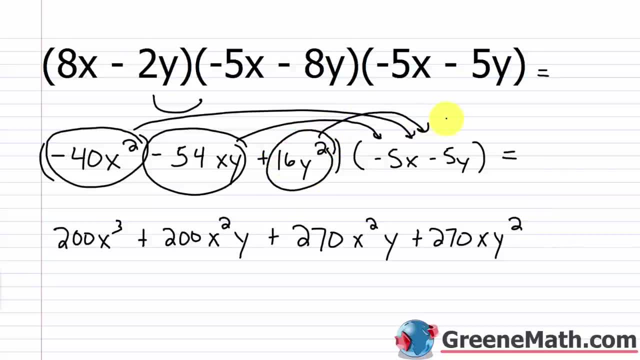 Now I'm going to take this guy and multiply it by this polynomial. So 16y squared times negative 5x. 16 times negative 5 is negative 80. 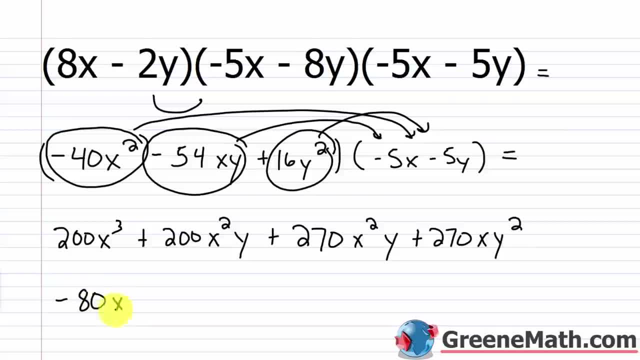 So that's negative 80. And then xy squared. And then 16y squared times negative 5y. That's negative 80y cubed. All right, then this equals, so 200x cubed. 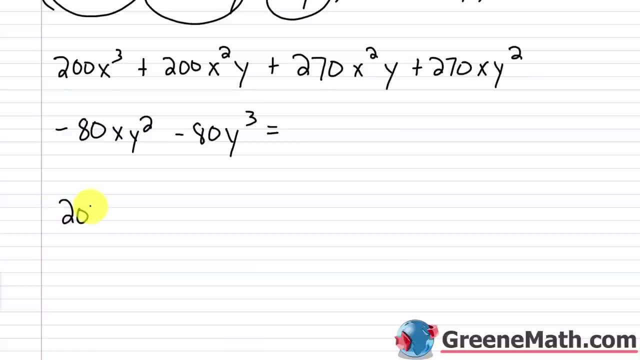 And then let's take a look at this. We have x squared y, x squared y. 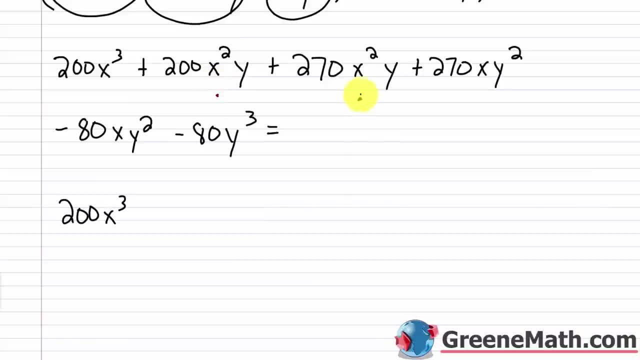 So no other like terms. Remember, for you to have like terms, it's got to be the same variable raised to the same power. So I've got to have an x squared and then a y to the first power. So that occurs here and here. Doesn't occur here. Doesn't occur here. 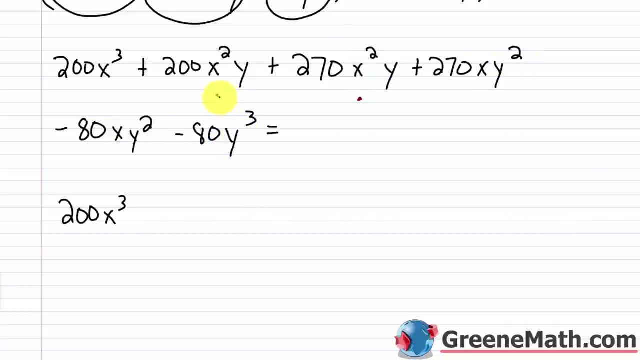 Doesn't occur here or here. So just these two are like terms. 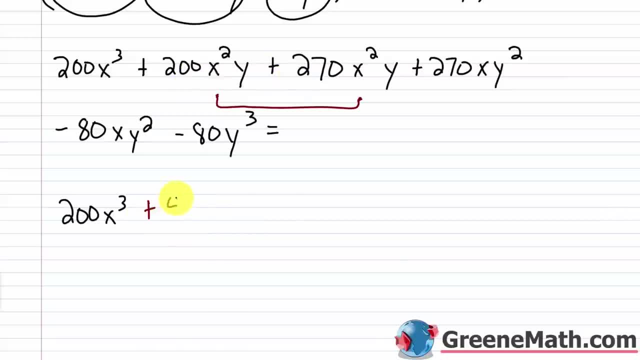 So 200 plus 270 is 470. And then x squared y. Now I have 270xy squared and negative 80xy squared. So these are like terms. These and only these can be combined together. 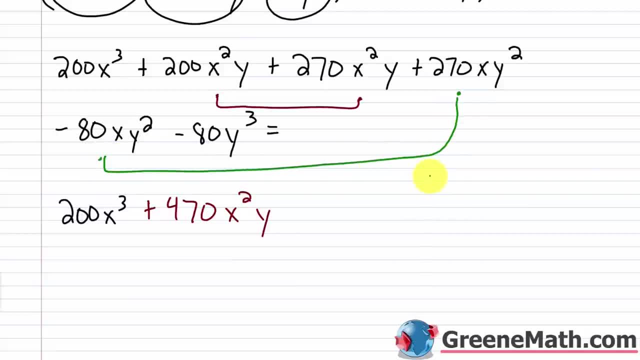 So 270 minus 80 is 190. So this would be plus 190xy squared. And then lastly I have minus, minus 80y cubed. Nothing I can combine with that. So my answer here is 200x cubed plus 470x squared y plus 190xy squared minus 80y cubed. 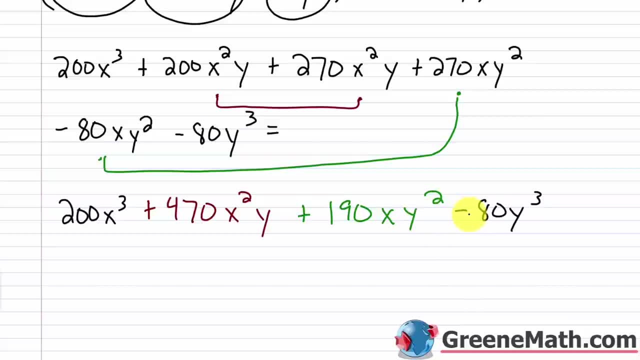 Hello and welcome to Algebra 1 Lesson 32. In this video, we're going to learn about special products. So you might see the title of this lesson 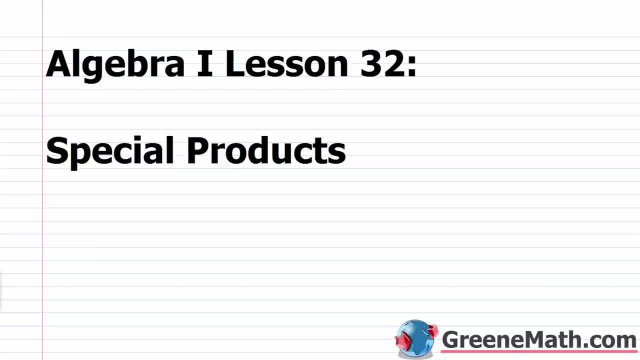 Hello and welcome to Algebra 1, Lesson 32.. In this video we're going to learn about special products. So you might see the title of this lesson and say: what do we mean by special products? Well, essentially, in this section, 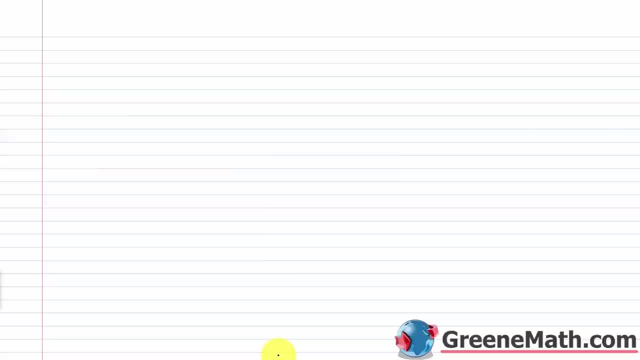 I'm going to give you some shortcuts for common binomial products. This is going to be a huge time saver for you moving forward. So I'm going to start out by just defining again what a binomial is. A binomial is a polynomial with two terms, So something generic like, let's say, x plus y. 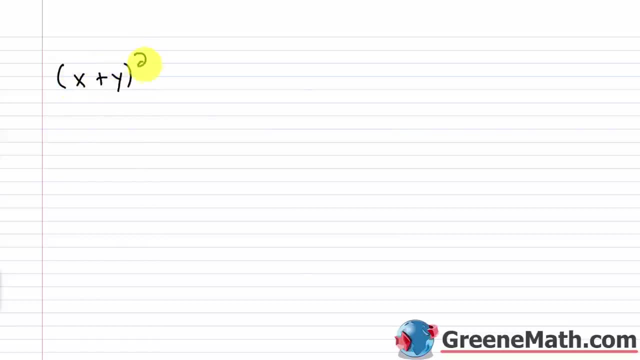 Okay, and let's say we squared this guy. Okay, let's say we squared this guy. What is this equal to? If I said: give me an answer for this, give me a value for this, what would you say? Well, a lot of students make the mistake of just trying to distribute. 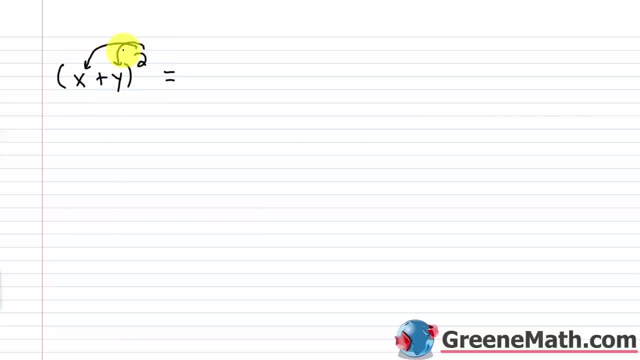 this exponent 2 to each term inside the parentheses, They say: okay, well, this is x squared plus y squared. That's a very, very common mistake in algebra and this is wrong. This is not the right answer. Okay, and to understand why this is wrong, why it's not the right answer: 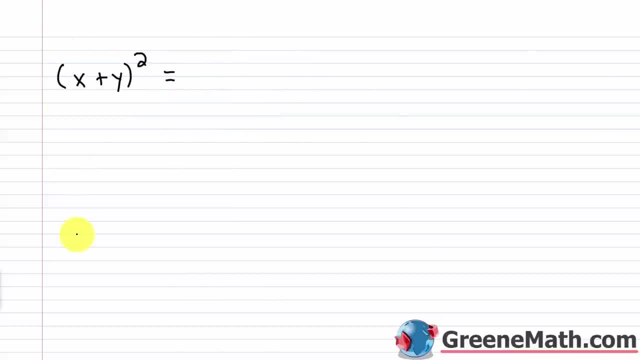 let's go back to the definition of squaring something. Let's say I had the number 4 and I want to square 4.. Well, what does this mean? It means I take this base 4 and I multiply it by itself, or I take the base 4 and I have two factors of 4.. So this is 4 times 4 or 16.. 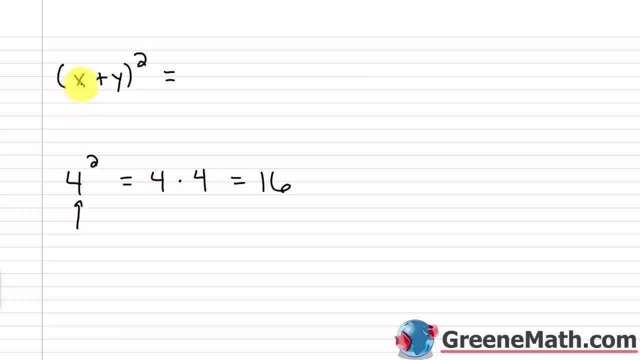 Well, by that same logic, if I have this quantity here, x plus y, and it's squared well, the base x plus y needs to be multiplied by itself. So this is x plus y times, x plus y. Right, I have two factors. my exponent is 2,. 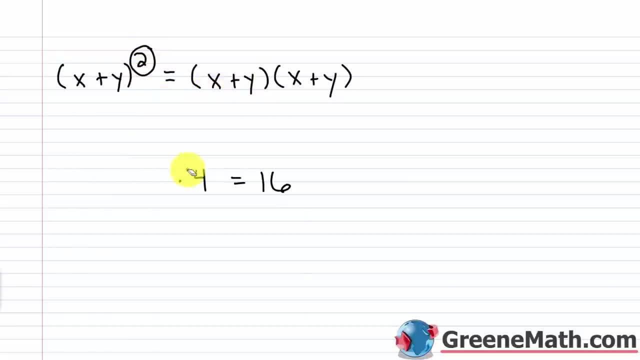 of x plus y. If I changed that exponent up and I said I have x plus y to the third power or cubed, well then I'd have three factors of x plus y. You've got to expand this out. Very, very important that you understand that moving. and say, what do we mean by special products? Well, we're going to learn about special products. 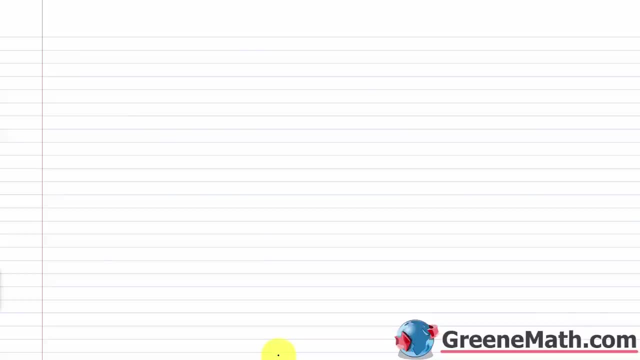 So you might see the title of this lesson and say, what do we mean by special products? 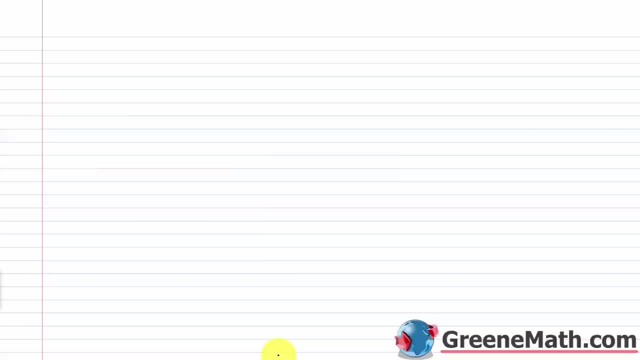 Well essentially in this section, I'm going to give you some shortcuts for common binomial products. 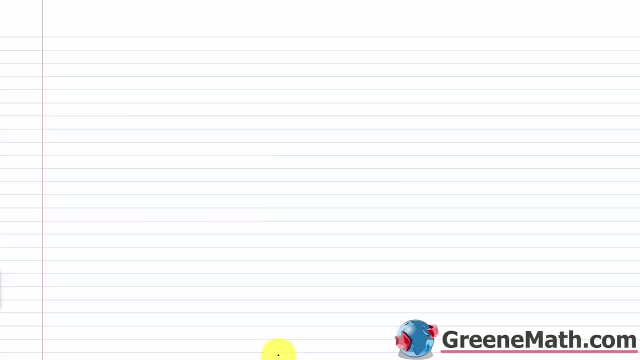 This is going to be a huge time saver for you moving forward. 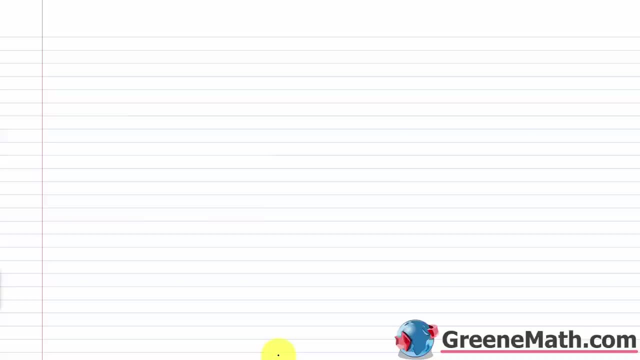 So I'm going to start out by just defining again what a binomial is. A binomial is a polynomial with two terms. So something generic like let's say x plus y. 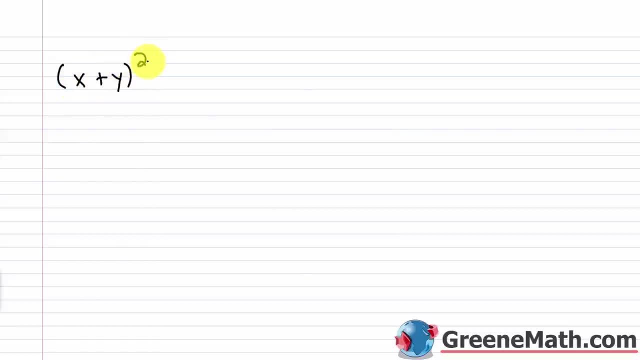 And let's say we squared this guy. 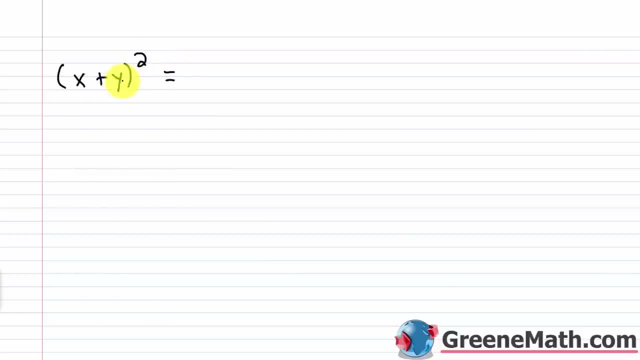 What is this equal to? If I said give me an answer for this, give me a value for this, what would you say? 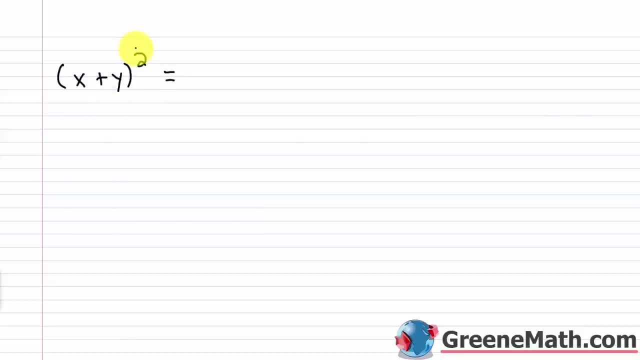 Well a lot of students make the mistake of just trying to distribute this exponent 2 to each term inside the parentheses. 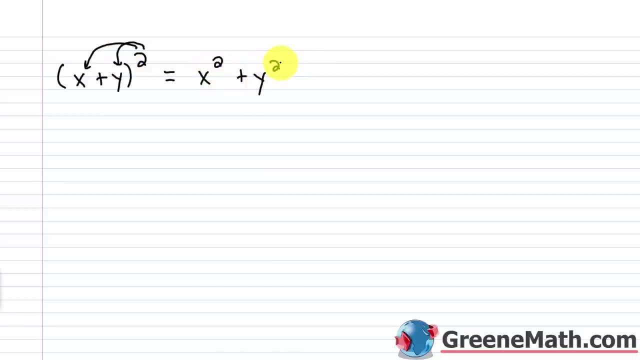 They say, well this is x squared plus y squared. That's a very, very common mistake in algebra. 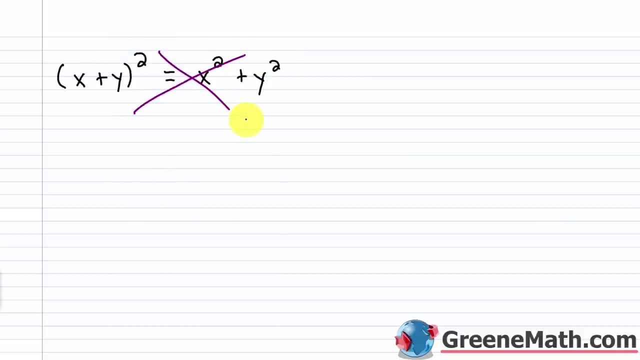 And this is wrong. This is not the right answer. 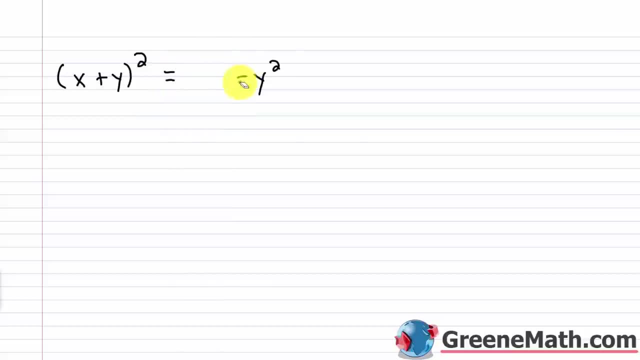 And to understand why this is wrong, why it's not the right answer, let's go back to the definition of squaring something. 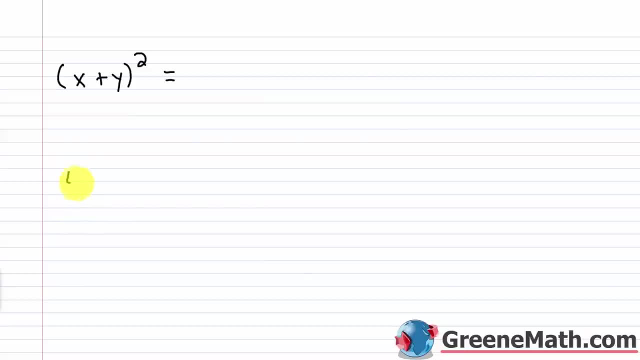 Let's say I had the number 4. And I want to square 4. Well what does this mean? It means I take this base 4 and I multiply it by itself. Or I take the base 4 and I have two factors of 4. So this is 4 times 4, or 16. 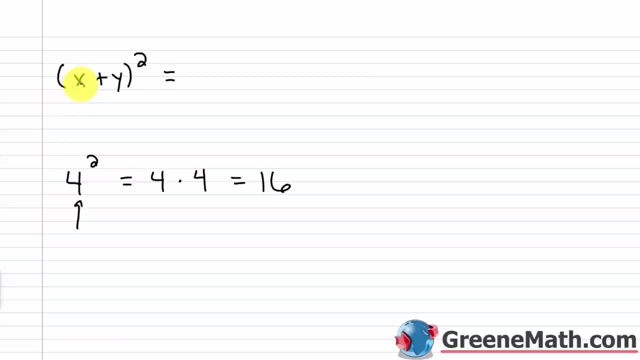 Well by that same logic, if I have this quantity here, x plus y, and it's squared, well the base, x plus y, needs to be multiplied by itself. So this is x plus y times x plus y. Right, I have two factors, my exponent is 2, of x plus y. 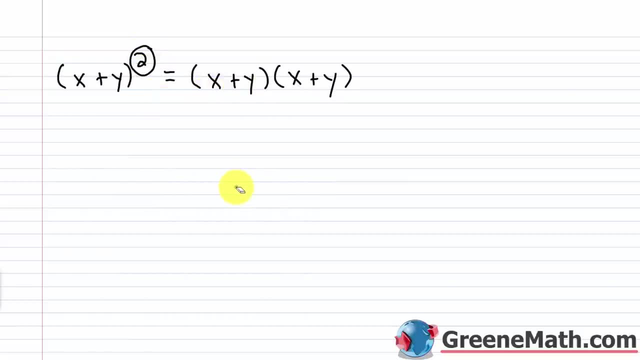 If I changed that exponent up and I said I have x plus y to the third power, or cubed, well then I'd have three factors of x plus y. 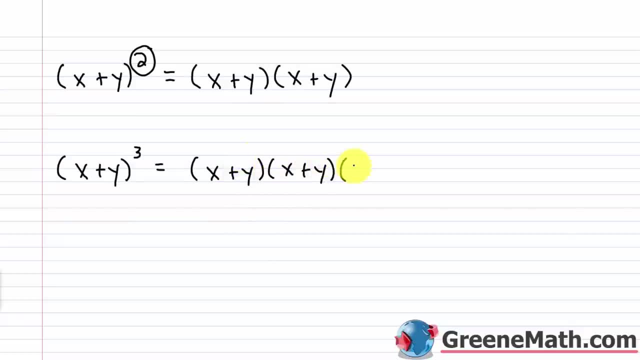 Right, you've got to expand this out. Very, very important that you understand that moving forward. 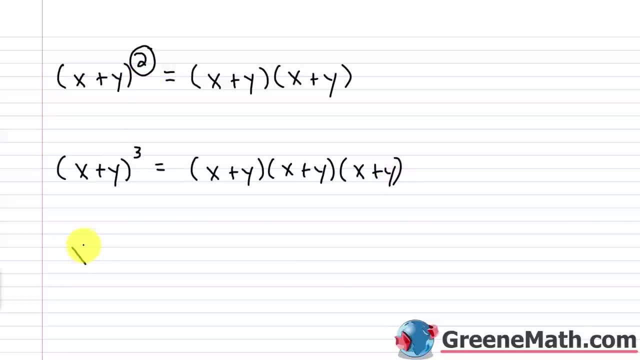 Because again, trying to say that x plus y, 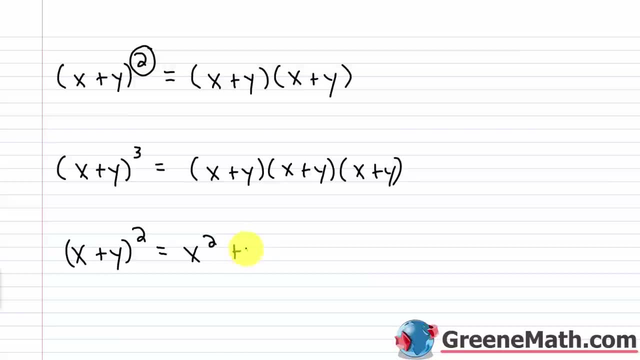 that quantity squared, is equal to x squared plus y squared, again, this is a very, very common mistake. 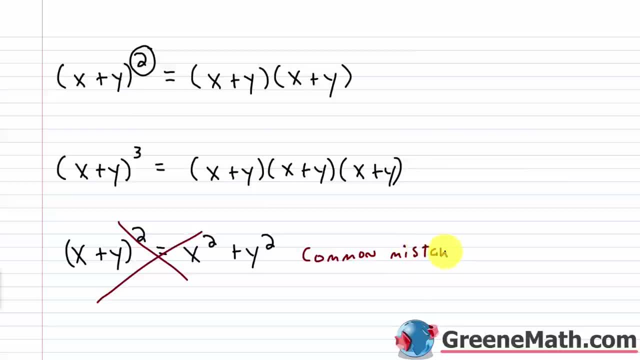 Common mistake. So now that we understand the basic logic behind 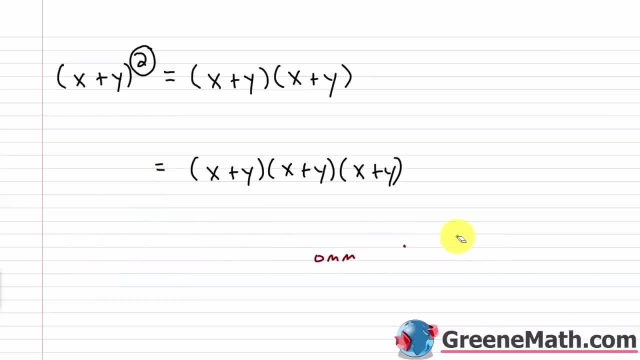 squaring a binomial, let's talk about how we can kind of get a generic formula going and speed our work up. 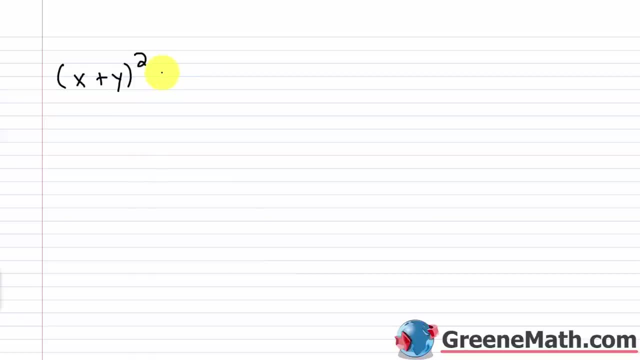 So if we know that x plus y, that quantity squared, again, is equal to x plus y times x plus y, 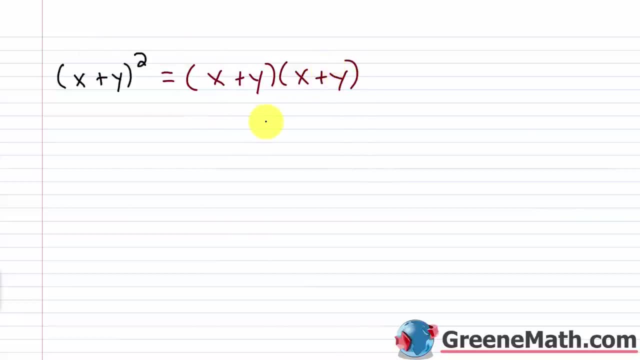 let's go through and use FOIL, remember we can use that to get the product of two binomials, to get our answer. 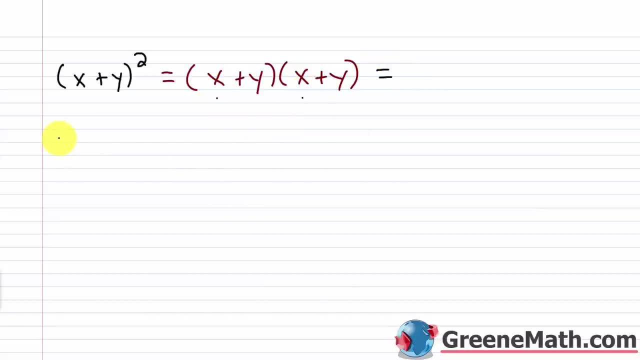 We would do the first terms, so x times x, that's x squared. Then we would do the outside terms, so x times y, plus xy. 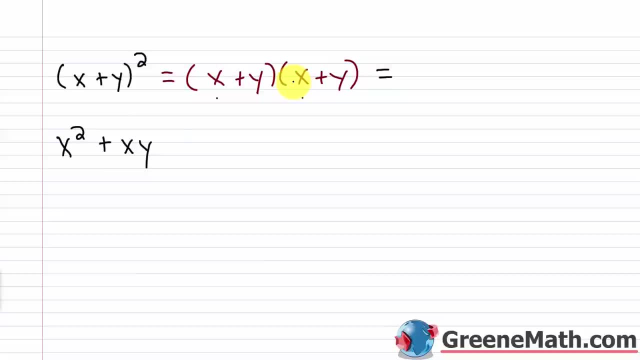 Then we would do the inside terms, y times x, which is yx or xy, doesn't matter, so plus xy. 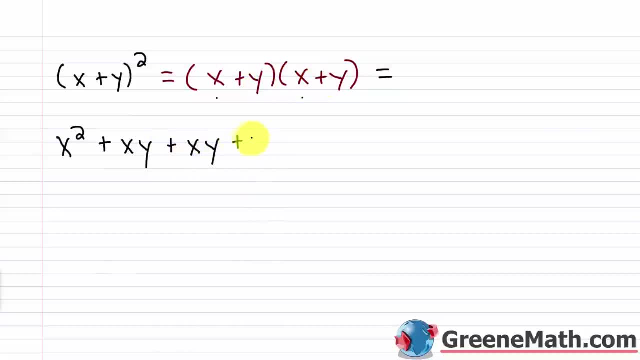 Then we would do the last terms, y times y is y squared, so plus y squared. 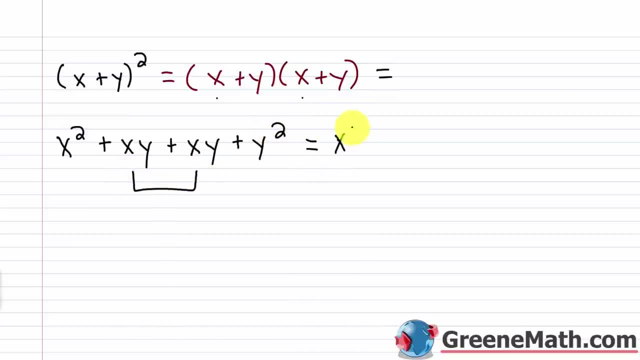 So if I combine like terms in the middle here, I'm going to end up with 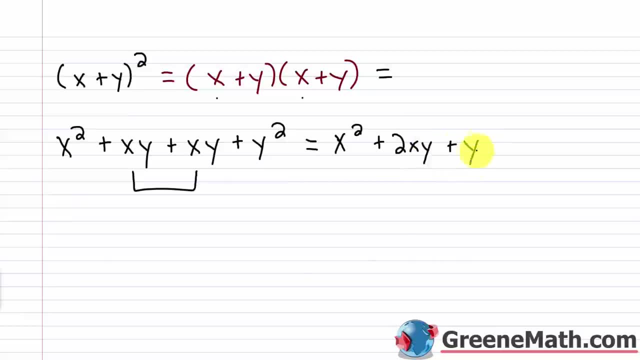 x squared plus 2xy plus y squared. 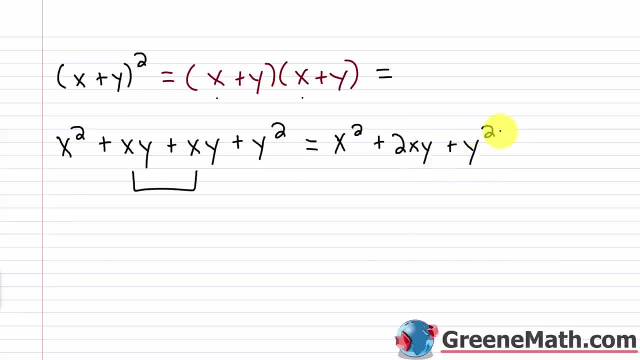 Now, this result is not unique. I can follow that same kind of format to get an answer when I have something that looks like this. 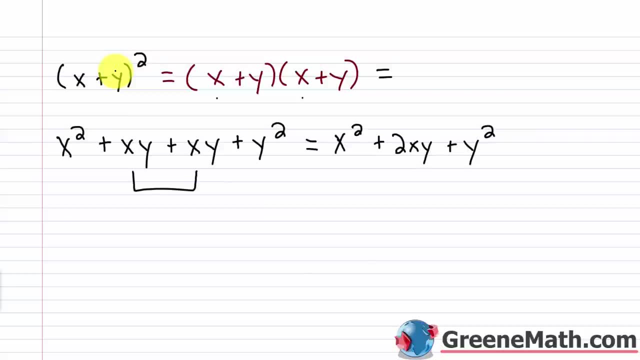 If I have a binomial that's squared, I'm always going to end up with the first term squared, here I have x as the first term, that ends up squared, plus 2 times the first term times the second term, so we have 2 times the first term x times the second term y, and then plus the final or last term squared. 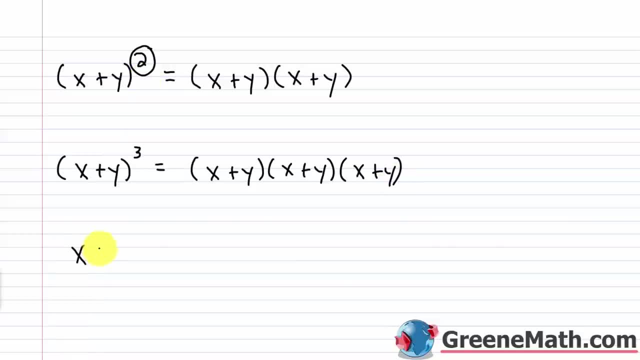 forward, because, again, trying to say that x plus y, that quantity squared is equal to x squared plus y squared, Again, this is a very, very common mistake, Common mistake. So now that we understand the basic logic behind squaring a binomial, let's talk about how we can. 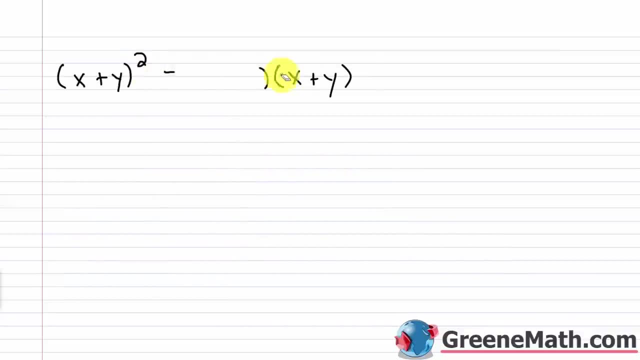 get a generic formula going and speed our work up. So if we know that x plus y, that quantity squared again is equal to x plus y times x plus y, Let's go through and use FOIL, Remember we can use that to get the product of two binomials. to get our answer We would do the first terms, so x times x. 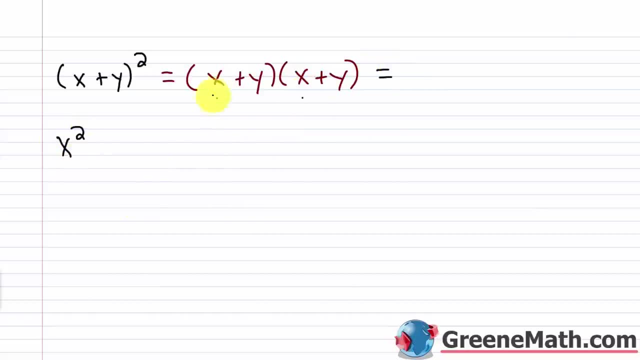 that's x squared, Then we would do the outside terms. so x times y, that's plus xy. Then we would do the inside terms: y times x. which is y, x or x, y, doesn't matter. so plus x, y, then we do the last terms. 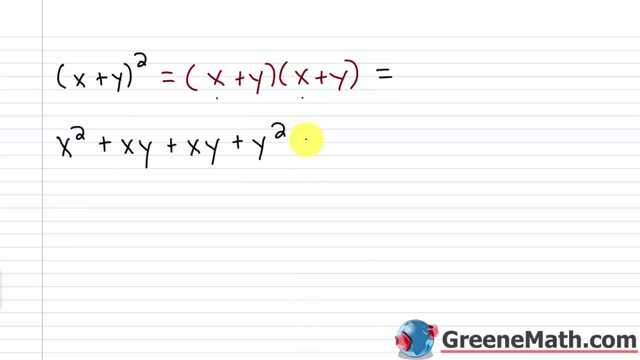 y times. y is y squared, so plus y squared. so if i combine like terms in the middle here, i'm going to end up with x squared plus 2xy plus y squared. now this result is not unique. i can follow that same kind of format to get an answer when i have something that looks like this: if i have a binomial: 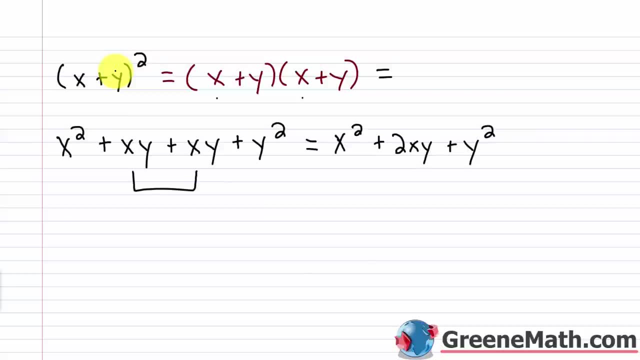 that's squared. i'm always going to end up with the first term squared. okay, here i have: x is the first term, that ends up squared, plus two times the first term, times the second term. so we have two times the first term, x times the second term, y, and then plus the final or last term. 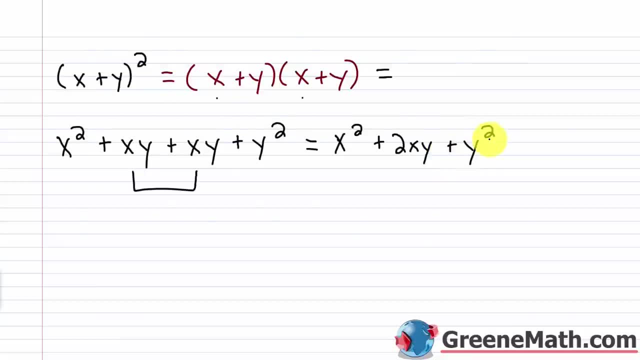 squared right. in this case i have y, so y is squared. you can kind of see- i've written this out here- the square of a binomial. we have x plus y, that quantity squared. you can kind of see, i've written this out here- the square of a binomial. we have x plus y, that. 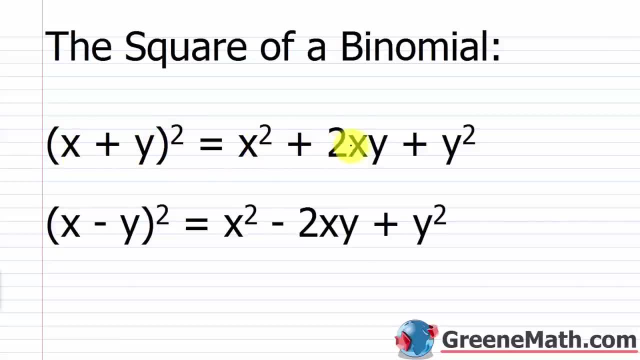 square of a binomial. we have x plus y, that quantity squared, and then plus the final or last term squared again. it follows this format: First term squared plus two times the first term, times the second term plus the final term or the last term squared. And you might not remember that right away, but In this case I have y, so y is squared. You can kind of see I've written this out here, the square of a binomial, we have x plus y, that quantity squared. 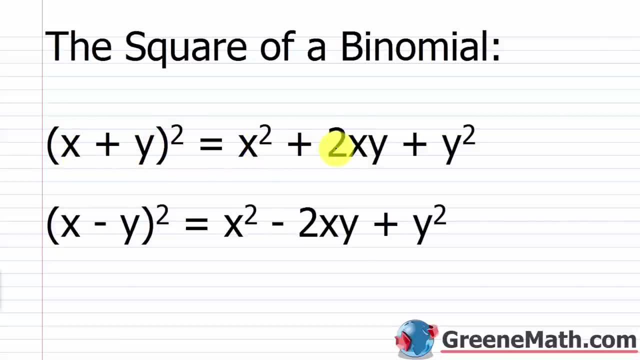 Again, it follows this format, first term squared plus 2 times the first term times the second term, plus the final term or the last term squared. 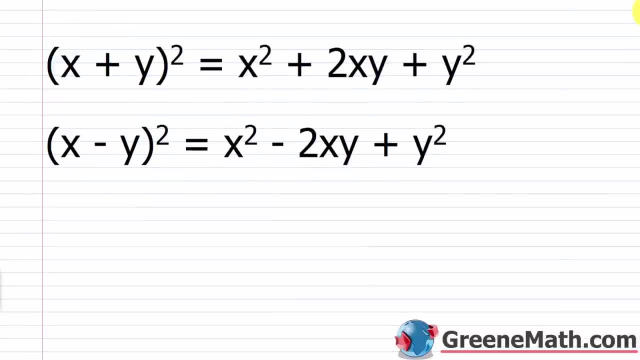 And you might not remember that right away, but you need to write that on a flash card and kind of write some notes on that and just keep looking at it over and over and over again, and this is going to be one of the things that saves you so much time. 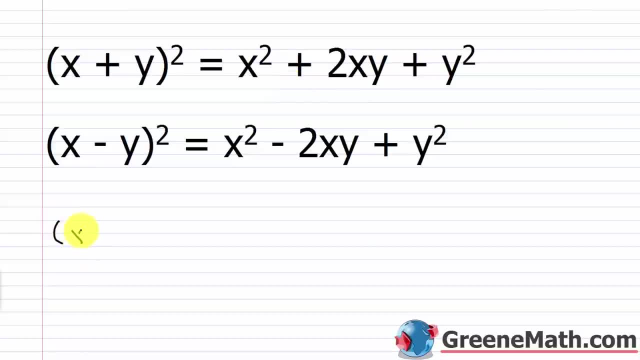 Let me give you an example. Let's say I just throw something at you like x plus 7, that's squared. Without doing FOIL, can you give me an answer? Well, I can get an answer just by, again, using the general formula. 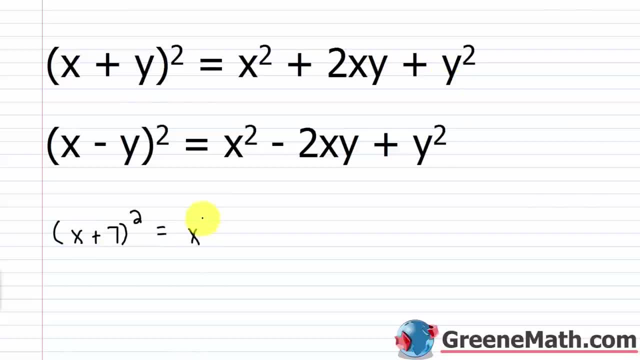 So I know it's the first term squared, so x squared, plus 2 times the first term times the second term or times the last term, so 2 times x times 7, 2 times 7 would be 14, so this would be 14x, and then plus the final term or the last term squared, 7 squared is 49. 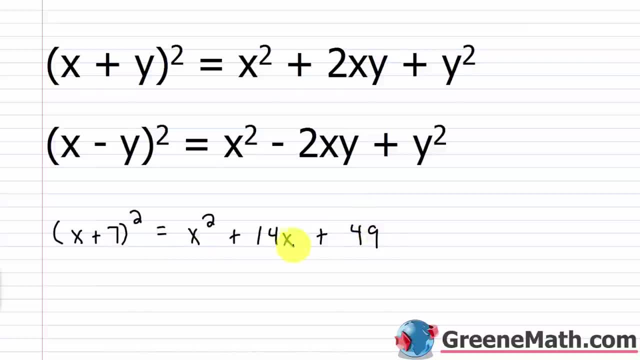 So without doing FOIL, I'm able to very quickly produce the result for the quantity x plus 7 squared. 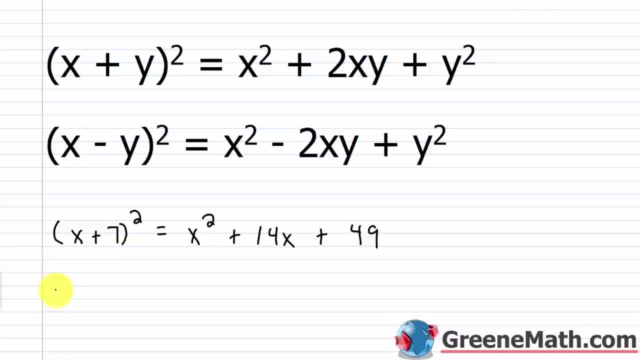 And if you don't believe that that works, let's expand this and I'll show you that I got the correct answer. 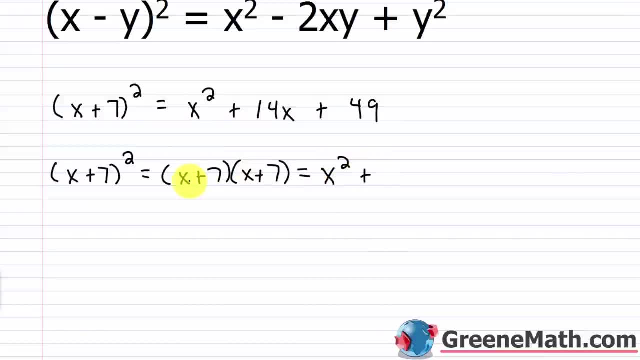 So x times x is x squared, plus x times 7, that's 7x, plus 7 times x, that's 7x again, plus 7 times 7, that's 49, and this equals x squared, plus combined like terms, 7x plus 7x is 14x, plus 49. 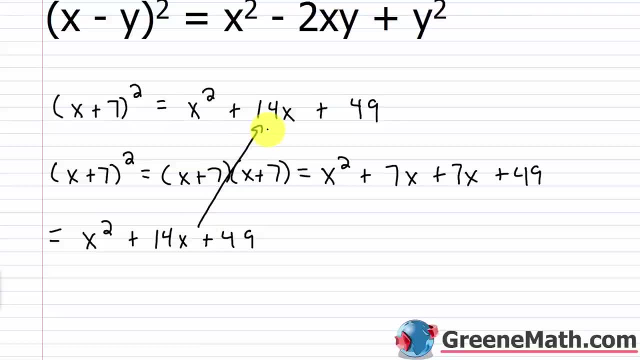 That's exactly what I got up here by just using that general formula. 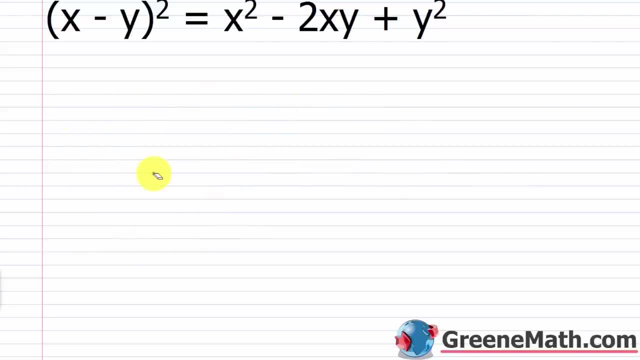 Now there's another one that we didn't look at yet, and the only difference between the one we looked at already and this one is that there's a minus sign. So there's a slight modification. 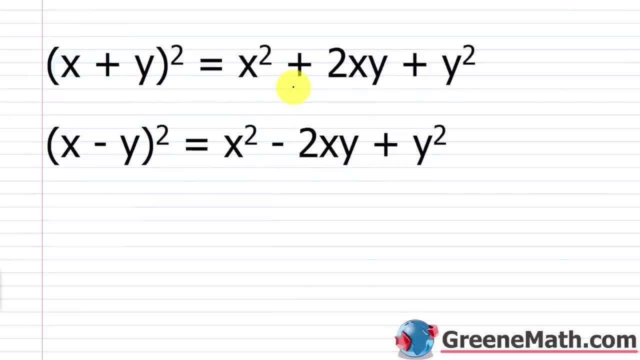 you need to write that on a flashcard and kind of write some notes on that and just keep looking at it over and over and over again, And this is going to be one of the things that saves you so much time. Let me give you an example. Let's say I just throw something at you like x plus seven. 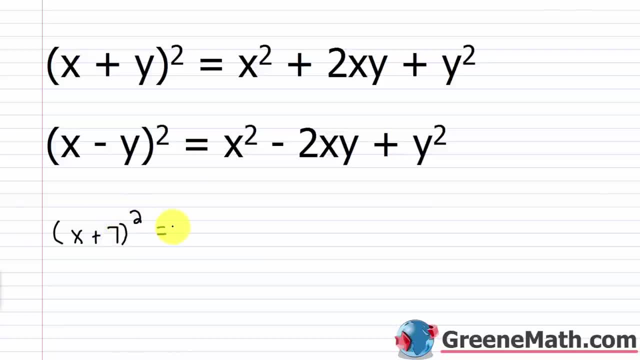 that's squared Without doing FOIL. can you give me an answer? Well, I can get an answer just by again using the general formula. So I know it's the first term squared, so x squared plus two times the first term, times the second term or times the last term, So two times x times seven. 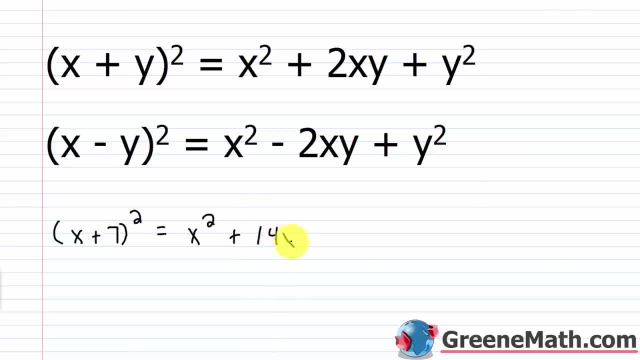 two times seven would be 14.. So this would be 14x, And then plus the final term, or the last term, squared Seven, squared is 49. So without doing FOIL, I'm able to very quickly produce the result for the quantity x plus seven. 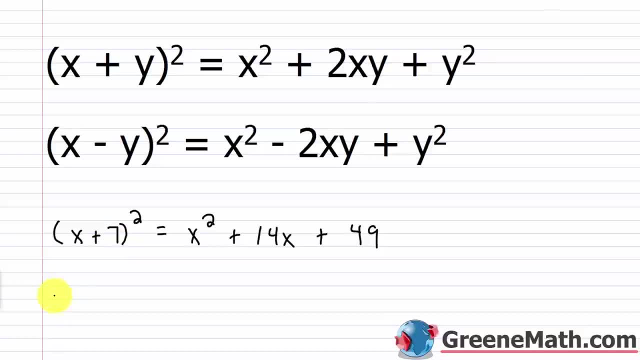 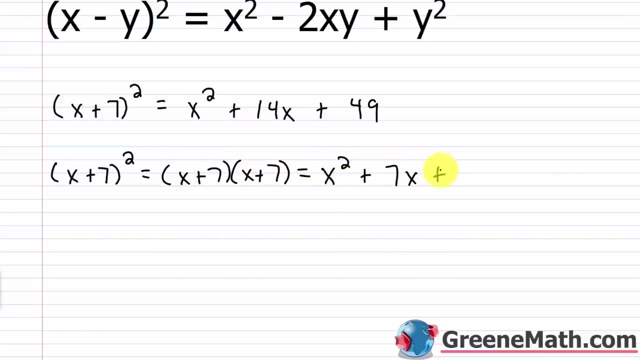 squared, And if you don't believe that that works, let's expand this and I'll show you that I got the correct answer. So x times x is x squared plus x times seven, that's seven x plus seven times x. 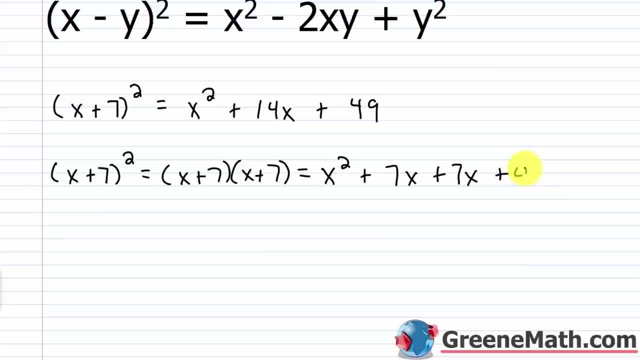 that's seven, x again plus seven times seven, that's 49.. And this equals, And this equals, And this equals: x squared plus combined like terms, seven x plus seven x is 14x plus 49. That's exactly what I got up here by just using that general formula. Now there's another one. 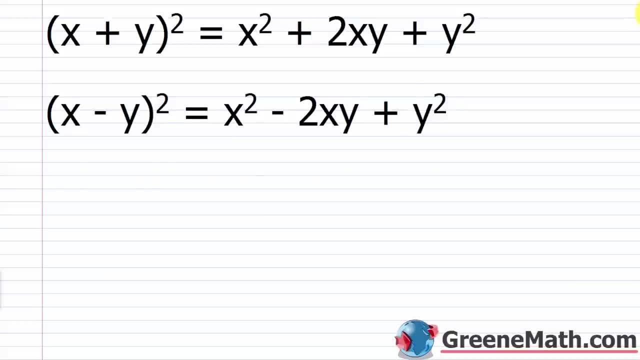 that we didn't look at yet, And the only difference between the one we looked at already and this one is that there's a minus sign. So there's a slight modification. It's the same thing to remember. It's just that there's a minus sign in front of the 2xy. So, for example, if I had something like 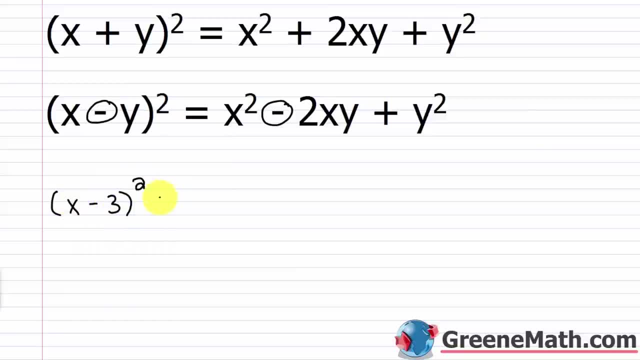 x minus three. that's squared. Well, following this formula, I would have x squared minus two times the first term, times the second term. So two times x times three would be six x, And then plus your second or your last term, squared Three, squared is nine. So I get x. 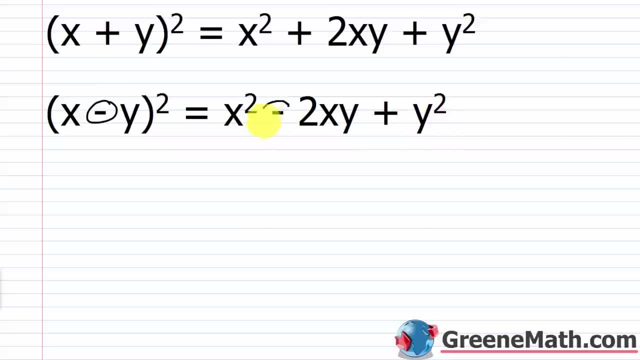 It's the same thing to remember, it's just that there's a minus sign in front of the 2xy. So for example, if I had something like 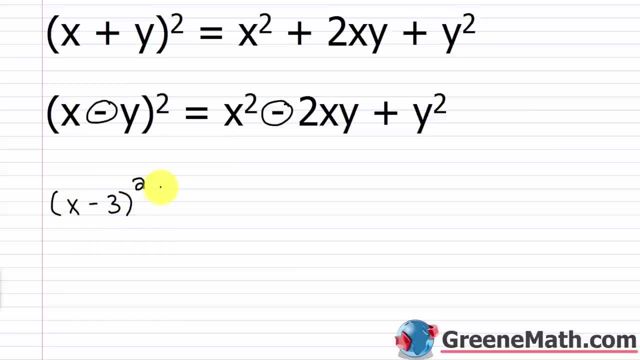 x minus 3, that's squared. 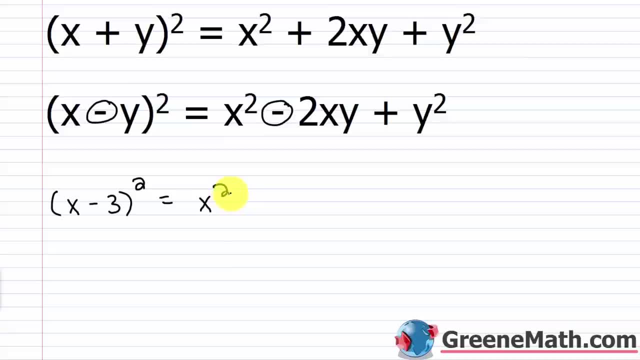 Well following this formula, I would have x squared minus 2 times the first term times the second term. 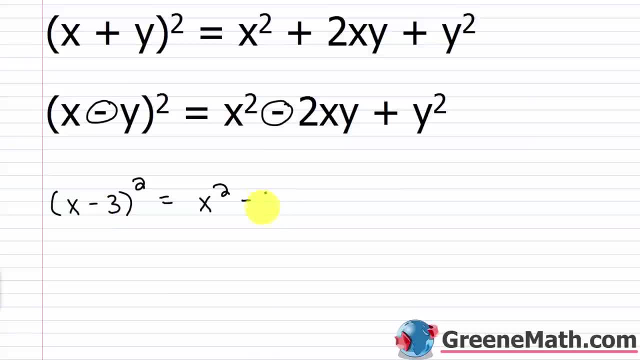 So 2 times x times 3 would be 6x, and then plus your second or your last term squared. 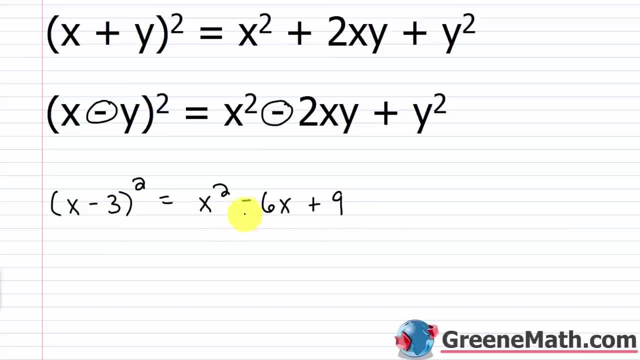 3 squared is 9. So I get x squared minus 6x plus 9. 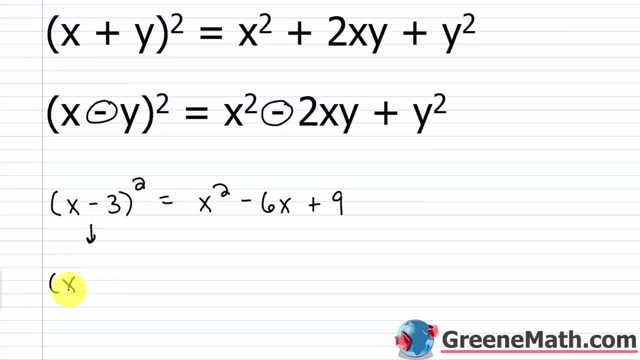 Now again, I could expand this, and show you kind of the slow way that I got the correct answer. 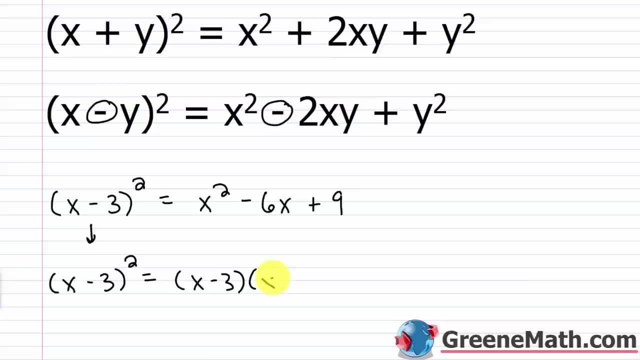 This is x minus 3 times x minus 3. So I get x squared, my first terms, and then x times negative 3 is negative 3x. Then negative 3 times x is negative 3x. Then negative 3 times negative 3 is plus 9. 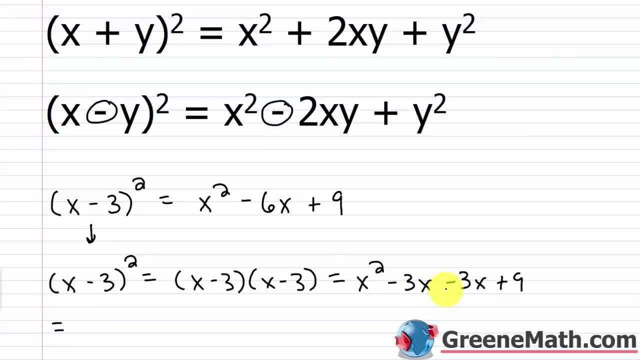 If I combine like terms here, negative 3x minus 3x is negative 6x. 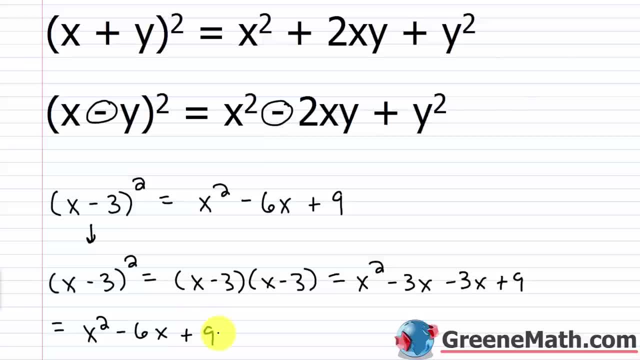 So I get x squared minus 6x plus 9. 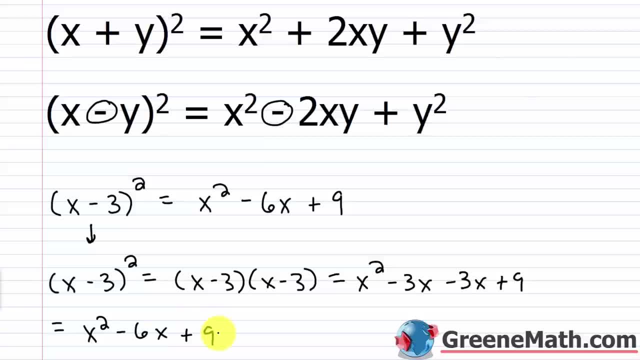 Now one thing I want to call your attention to, I get a lot of students that use this formula, and at first they're making sign mistakes. 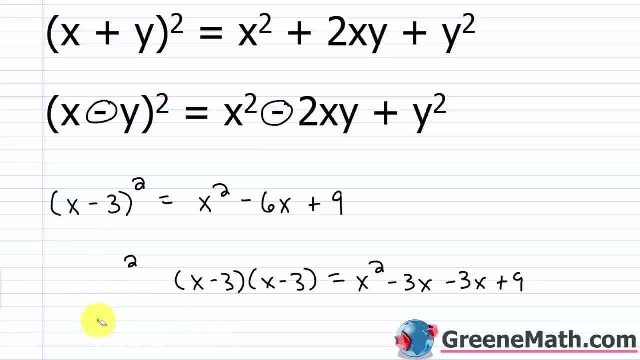 So what I want you to understand here, when you use this formula, the signs are already kind of calculated for you. 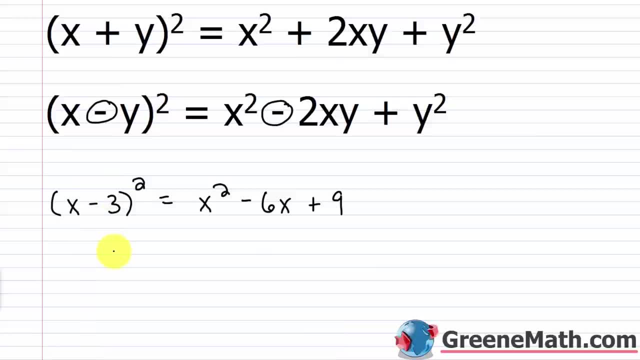 So don't worry about putting it in as negative 3. Just think about what number is here, and what number is here. Or it could be a variable or whatever you have. So whatever's in this position is here squared. Whatever's in this position and this position, don't worry about the sign. It's going to be 2 times this times this. 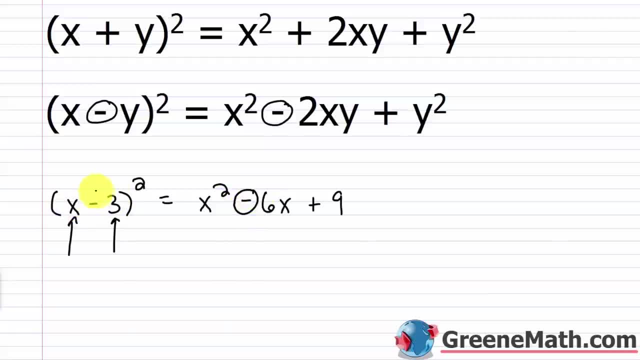 The sign comes into play here. So if this is a negative, you put a negative there. If it's a positive, you put a positive there. If this was a plus, I would just put a plus there. But don't go through and start thinking of this as negative 3 and jam up your multiplication and say, okay, well, I have 2 times x times negative 3. 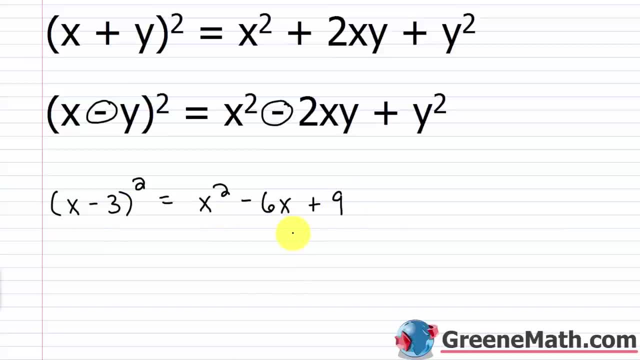 squared minus six, x plus nine. Now again I could expand this and show you kind of the slow way That I got the correct answer. This is x minus three times x minus three. So I get x squared by my first terms And then x times negative three is negative three x. Then negative three times x is. 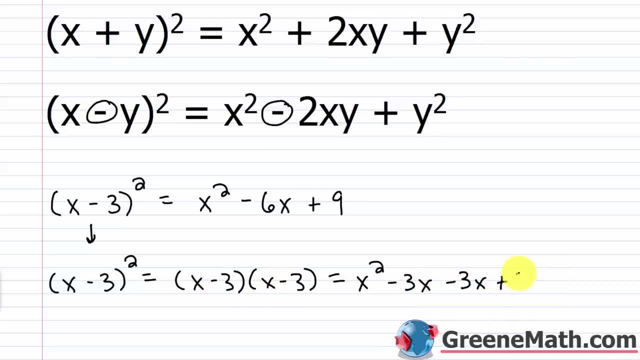 negative three x And then negative three times. negative three is plus nine. If I combine like terms here, negative three x minus three x is negative six x. So I get x squared minus six x plus nine. Now one thing I want to call your attention to. 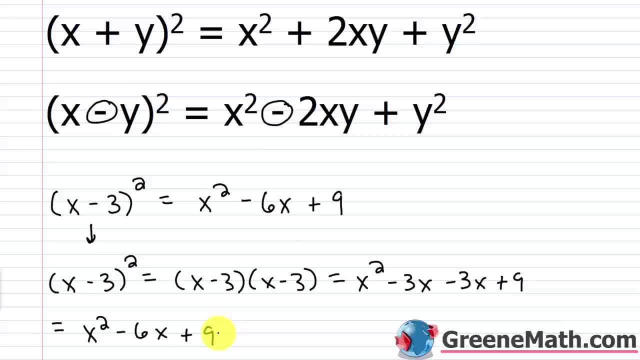 I get a lot of students that use this formula and at first they're making sign mistakes. So what I want you to understand here: when you use this formula, the signs are already kind of calculated for you. So don't worry about putting it in as negative three. Just think about what. 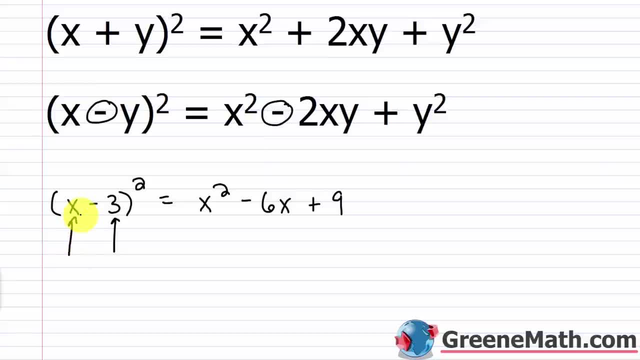 number is here and what number is here? Or it could be a variable, or whatever you have. So whatever's in this position is here squared. Whatever's in this position and this position, don't worry about the sign It's going to be. 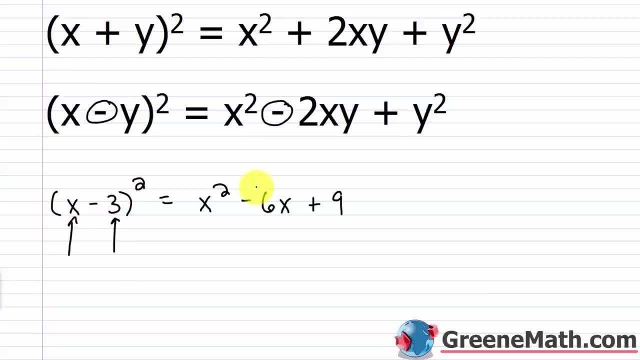 two times. this times this, The sign comes into play here. Okay, so if this is a negative, you put a negative there. If it's a positive, you put a positive there. right? If this was a plus, I would just put a plus there. But don't go through and start thinking of this as negative. 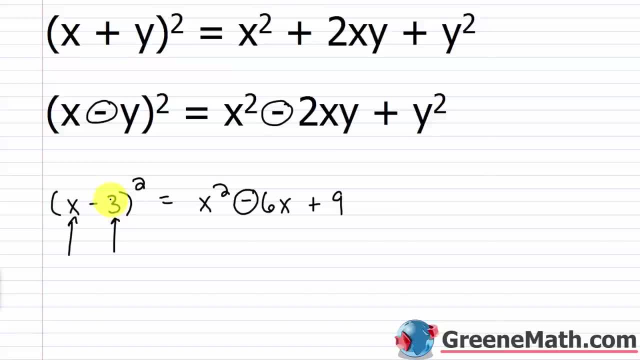 three and jam up your multiplication and say, okay, well, I have. you know, two times x, times negative three, you get negative six x. And then you put minus there from the formula, minus the negative six x, and you get plus six x. 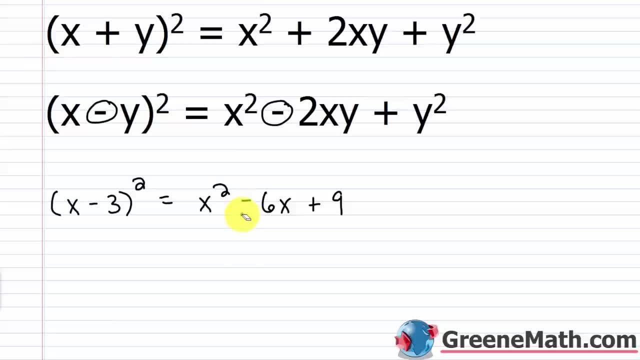 Please don't do that. The sign is already figured out for you. You just need to be very, very simple here and say: okay, I have this as my first value and this is my second value. Don't think about the sign, Just follow the general formula. All right, so let's do some. 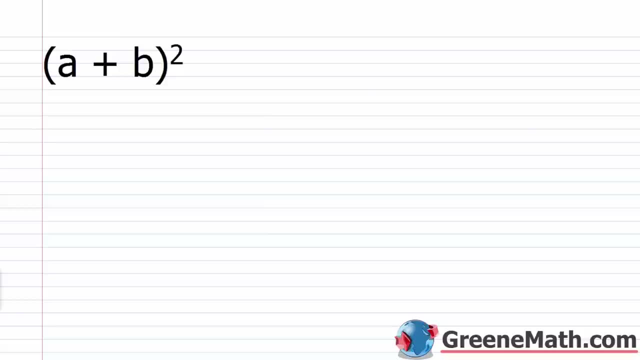 quick practice. We have this quantity a plus b, that's squared. So, again following the general formula, I know I'm going to take the first term and I'm going to square it. So a squared, then I have plus. I'm going to take two times the first term, times the second term, So two times a- b. 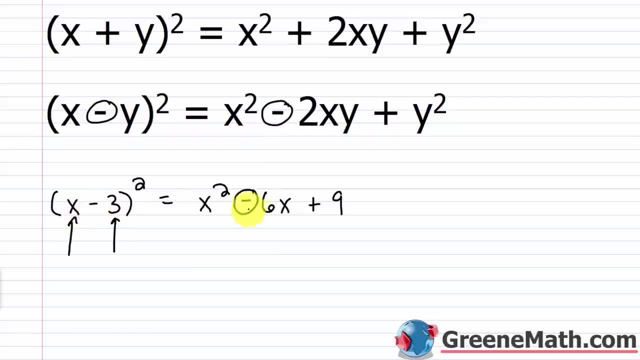 You get negative 6x. And then you put minus 6x. There's a plus there from the formula. 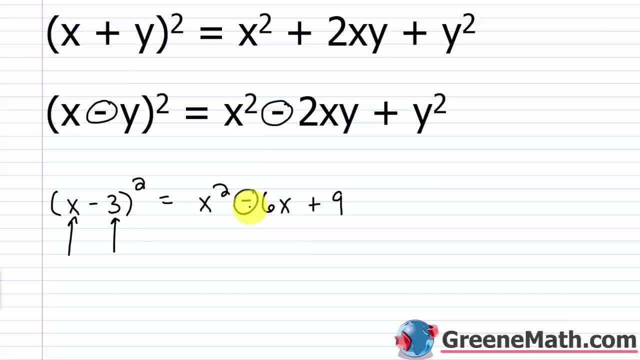 You put minus the negative 6x, and you get plus 6x. 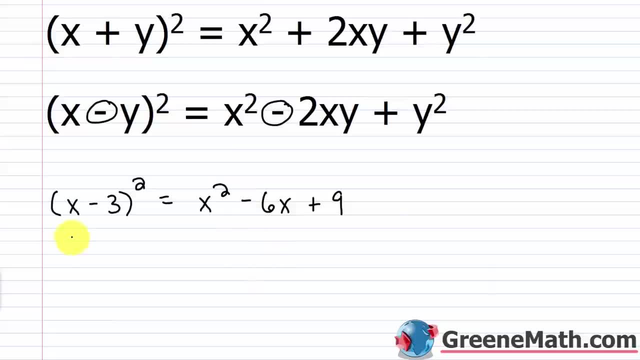 Please don't do that. The sign is already figured out for you. 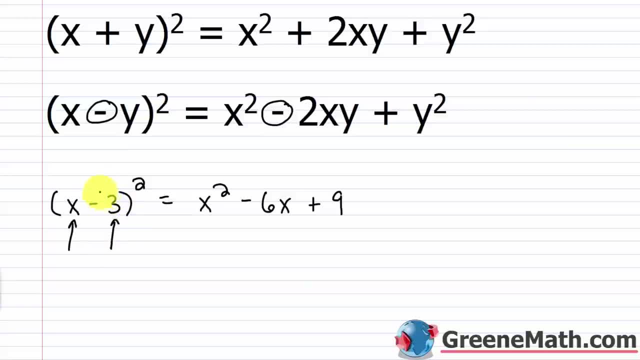 You just need to be very, very simple here and say, okay, I have this as my first value and this as my second value. Don't think about the sign. 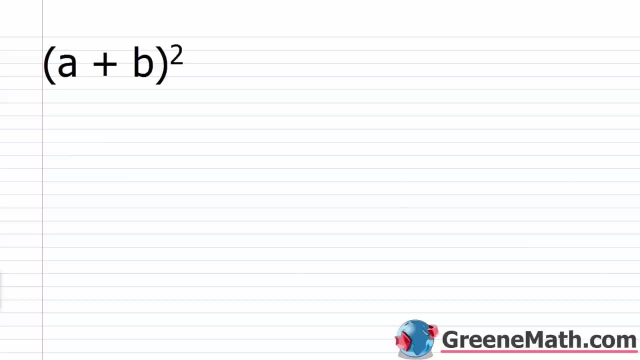 Just follow the general formula. All right, so let's do some quick practice. We have this quantity a plus b 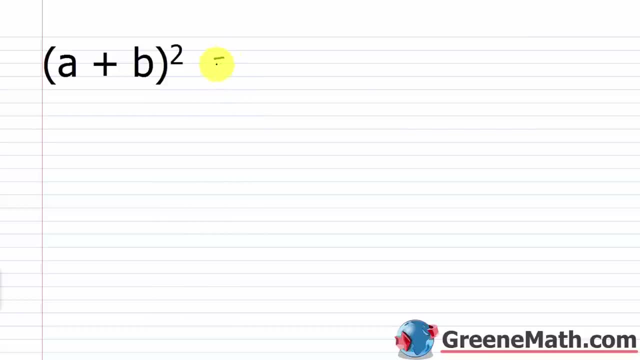 that's squared. So again, following the general formula, I'm going to take the first term and I'm going to square it. So a squared. 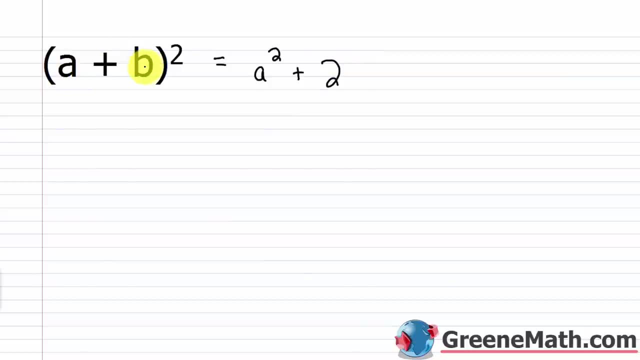 Then I have plus. I'm going to take 2 times the first term times the second term. So 2 times ab. Then plus. I'm going to have the last term squared. So plus b squared. 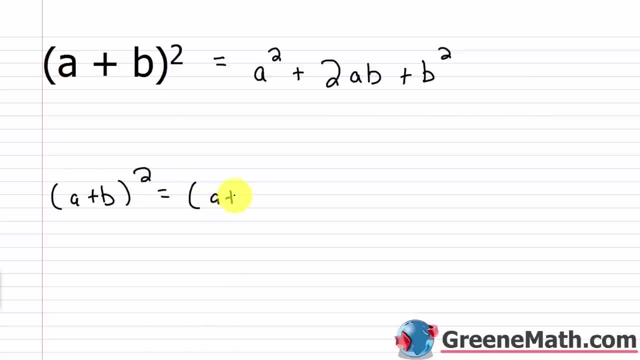 And again, you can check all of these. You just take this a plus b, this quantity squared, and you expand it. 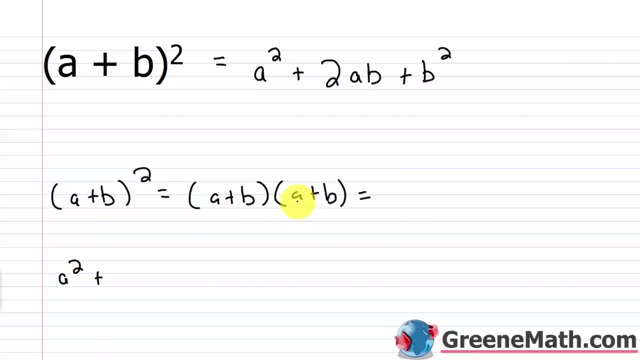 a plus b times a plus b. Plus a times b is ab. Plus b times a is ab. Then lastly, b times b is b squared. 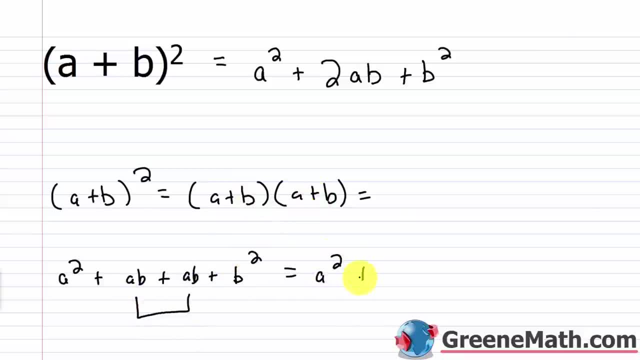 If I combine like terms here, I get a squared plus 2ab plus b squared, 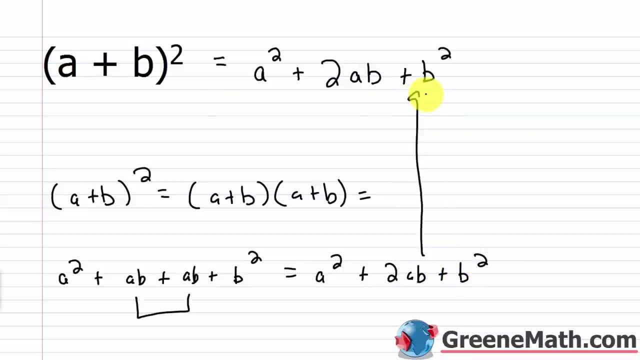 which is exactly what I had right then. 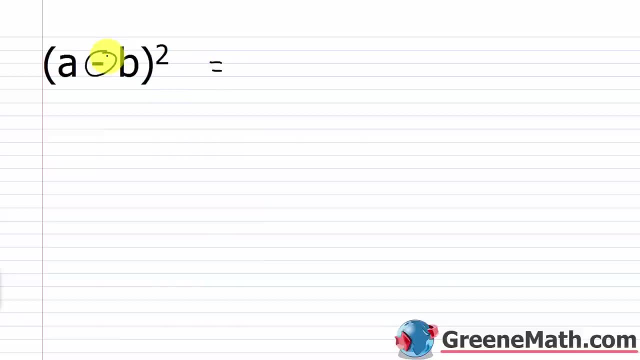 What about a minus b squared? Again, the only difference is going to be that sign there. So I'm going to have the first term, which is a squared, then minus, right, because of that sign, plus the first term, which is a, times the second term, which is b, and then plus the second term squared. 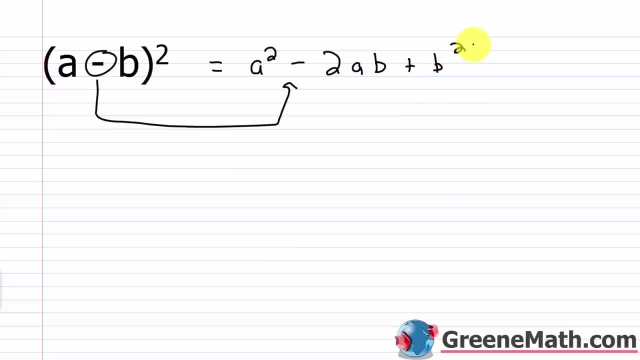 So b squared. So a squared minus 2ab plus b squared. 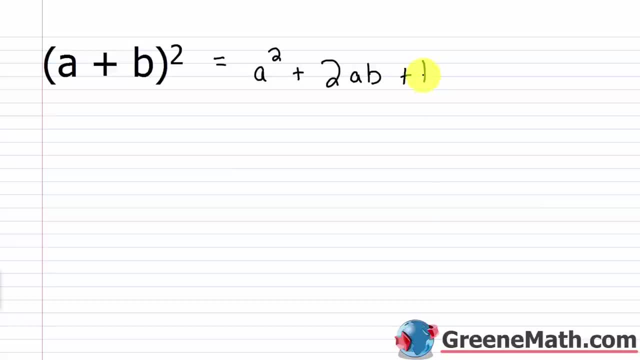 then plus- I'm going to have the last term- squared, So plus b squared. And again, you can check all of these. You just take this a plus b, this quantity squared, and you expand it: a plus b. times a plus b. This equals a times a is a squared plus a. times b is a b plus b. times a is a. 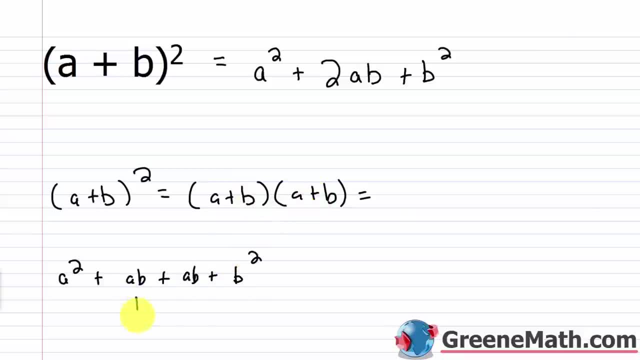 squared. Then, lastly, b times b is b squared. If I combine like terms here, I get a squared plus two, a b plus b squared, which is exactly what I had right there. What about a minus b squared? Again, the only difference is going to be that sign there, So I'm going to have the first term. 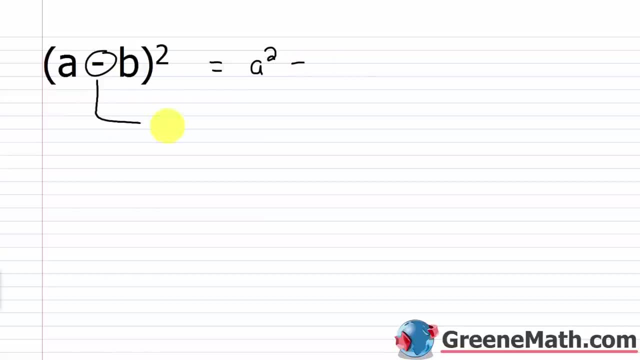 which is a, squared, then minus right because of that sign two times the first term, which is a, times the second term, which is b, and then minus right because of that sign b, and then plus the second term: squared, So b. squared, So a squared minus two: a, b plus b. 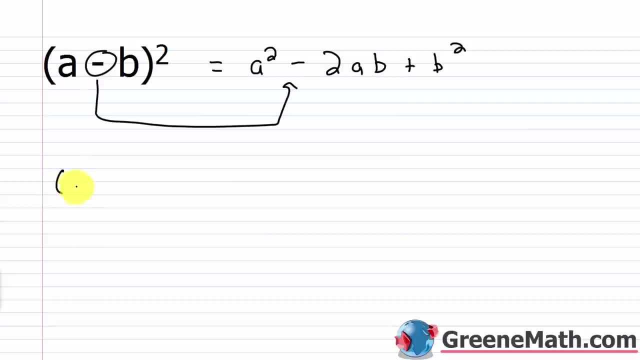 squared. And again, if you don't believe me, take this guy and go ahead and use FOIL to expand this right. It is a minus b times a minus b- and verify that this is exactly what you get. All right. here's something a little bit more typical, and this is where it's really going. 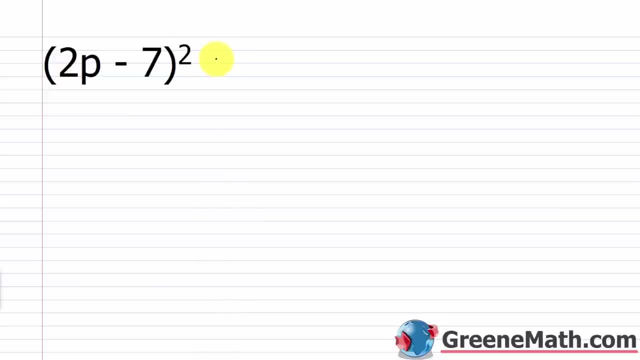 to save you the time. So I have two p minus seven, that quantity squared. So, using my formula, whatever's in the first position, that's this whole thing right here. okay, The two p is in the first position, That's my first term, So that's going to be squared. So. 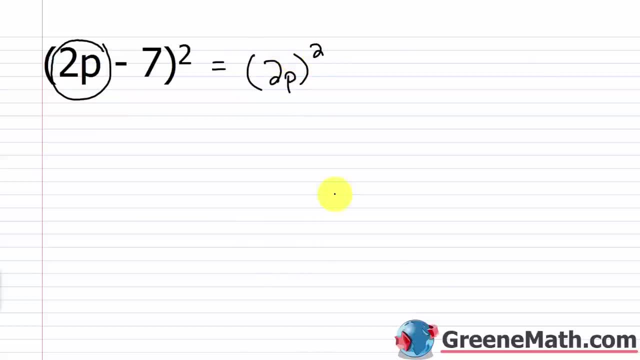 the two p is squared, And don't make the mistake of just writing two p squared. The whole thing is squared, So the two is squared and so is the p. So if I evaluate this, I would end up with what Two squared, which is four times p squared. 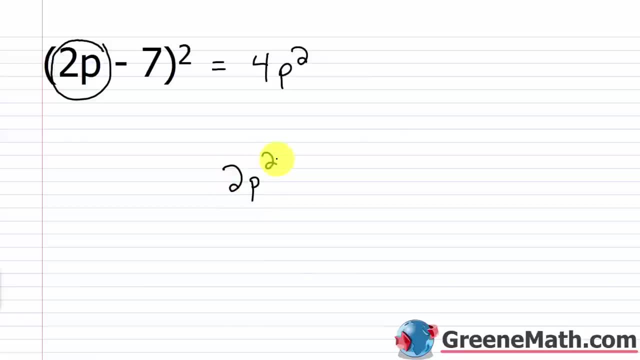 Another common mistake would be to say, okay, I just have two p squared. No, the whole thing has to be squared. Then I have the minus here and then times two times whatever's in this position. So that's times two p times whatever's in this position, which is seven. Two times two is four. Four times seven is 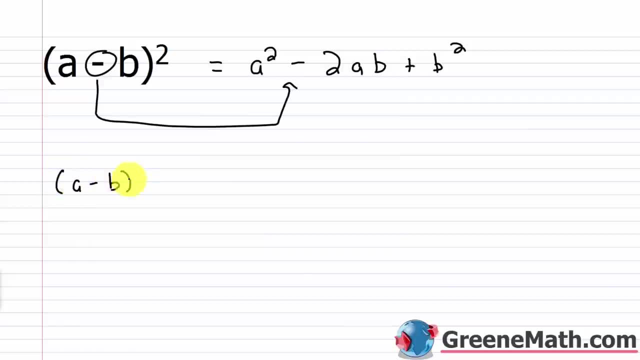 And again, if you don't believe me, take this guy and go ahead and use FOIL to expand this. It is a minus b times a minus b and verify that this is exactly what you get. 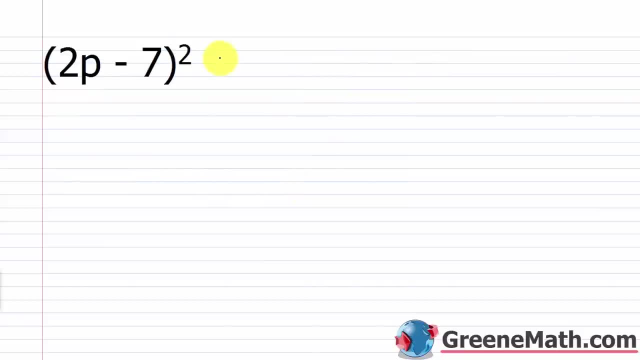 Alright, here's something a little bit more typical, but I'm going to save you the time. 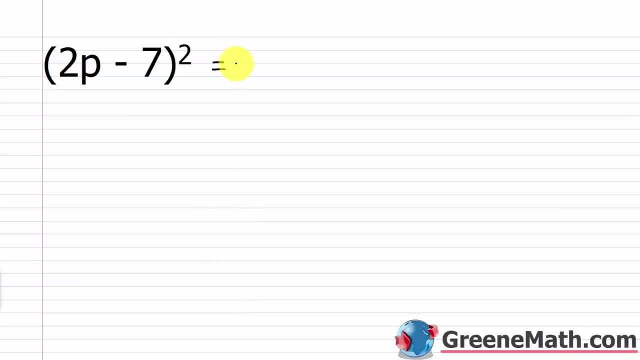 So I have 2p minus 7, that quantity squared. So using my formula, whatever's in the first position, that's this whole thing right here. The 2p is in the first position, that's my first term. 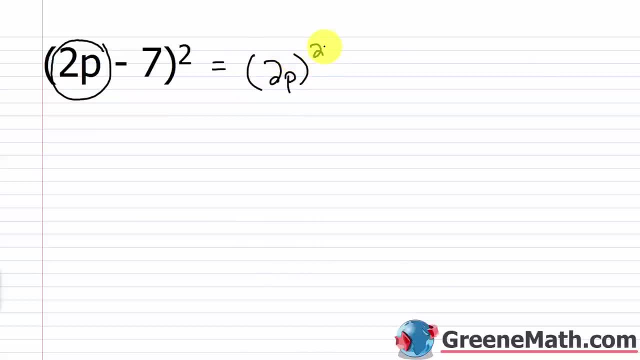 So that's going to be squared. So the 2p is squared. And don't make the mistake of just writing 2p squared. The whole thing is squared. 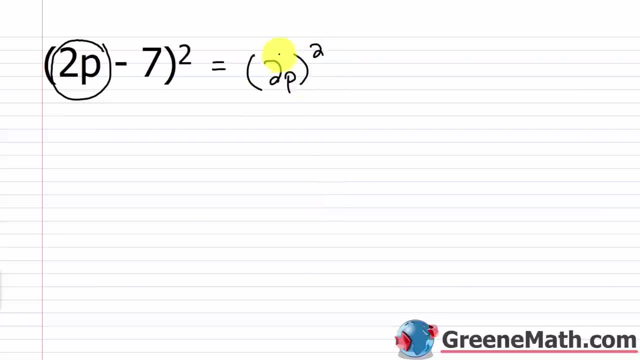 So the 2 is squared, and so is the p. So if I evaluate this, I would end up with what? 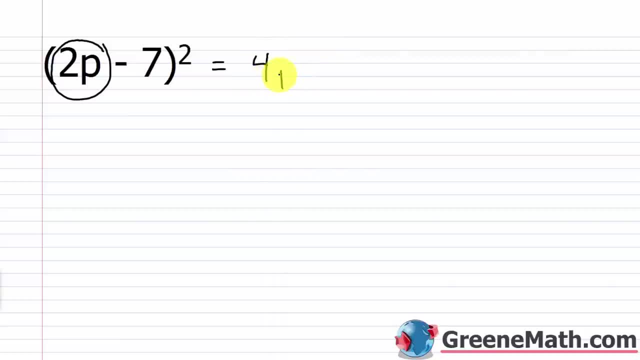 Which is 4 times p squared. 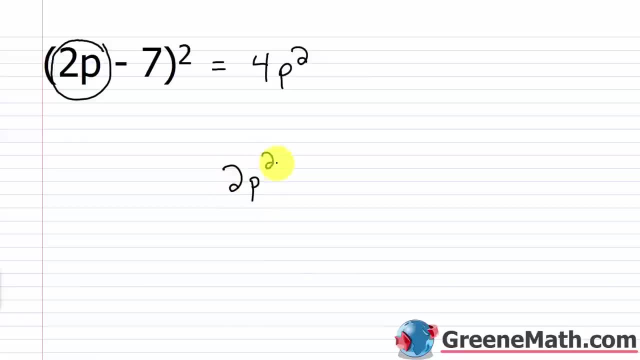 Another common mistake would be to say okay, I just have 2p squared. No. The whole thing has to be squared. 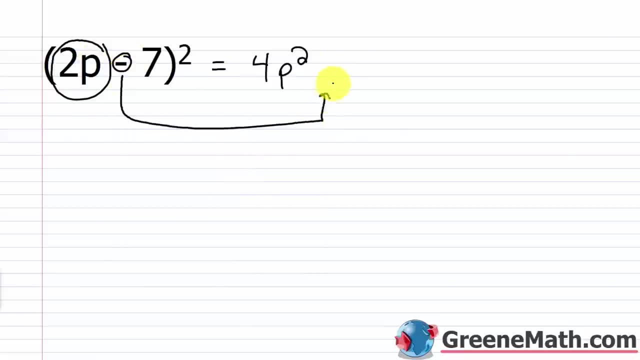 Then I have the minus here, and then times 2 times whatever's in this position, so that's times 2p, times whatever's in this position, which is 7. 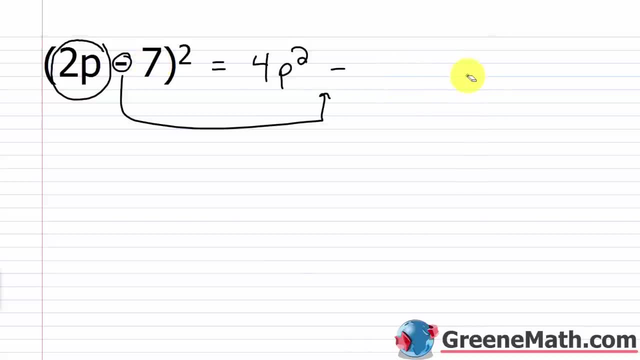 2 times 2 is 4, 4 times 7 is 28. So this would be minus 28p. 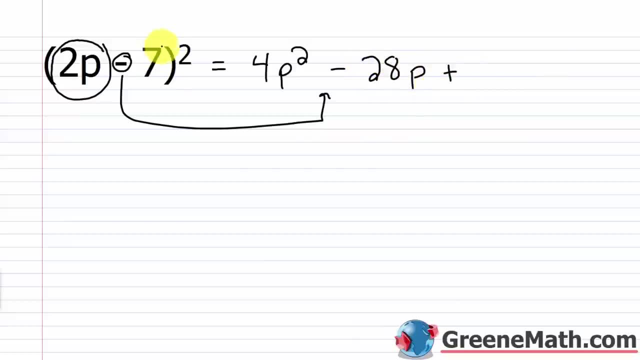 And then lastly, I'm going to add whatever's in this position squared. 7 times 7 is 49. So we end up with 4p squared minus 28p plus 49. Now again, this is one that I feel that we should check. 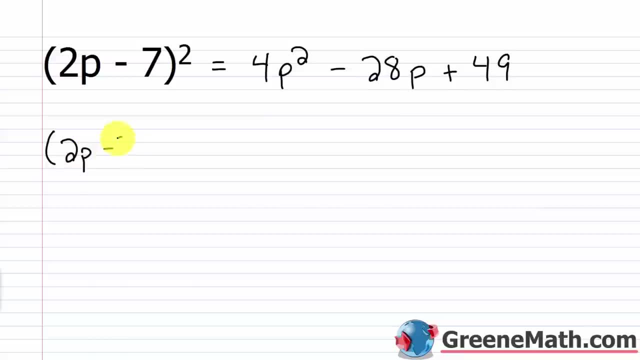 So I could show you we got the right answer. So we got 2p minus 7, that's squared. So this is going to expand out to 2p minus 7 times 2p minus 7. 2p times 2p. First terms. That's 4. 2 times 2 is 4. And then p times p is p squared. 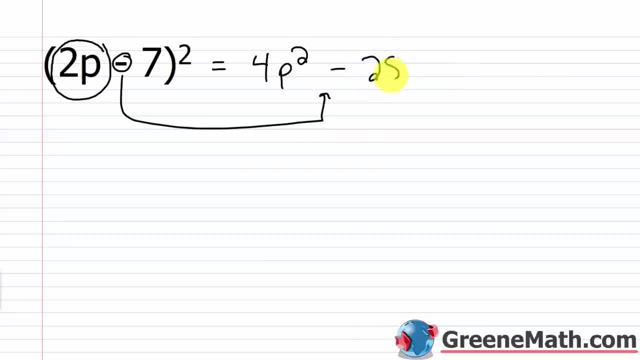 28.. So this would be minus 28 p. And then, lastly, I'm going to add whatever's in this position: squared Seven times seven is 49. So we end up with four p squared minus 28 p plus 49.. Now again, this is one. 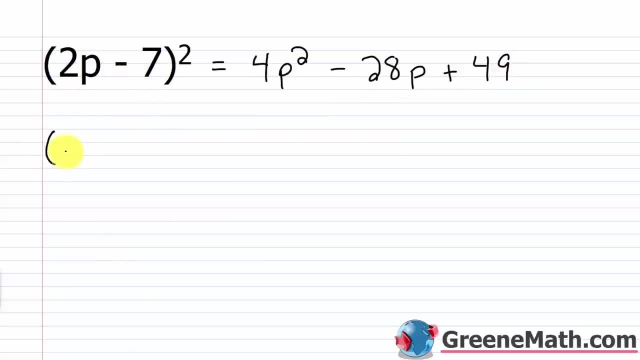 that I feel that we should check So I could show you we got the right answer. So we got two p minus seven, that's squared. So this is going to expand out to two p minus seven times two, p minus seven. Two p times two, p, first terms, That's four. Two times two is four, And then p times p is p squared. 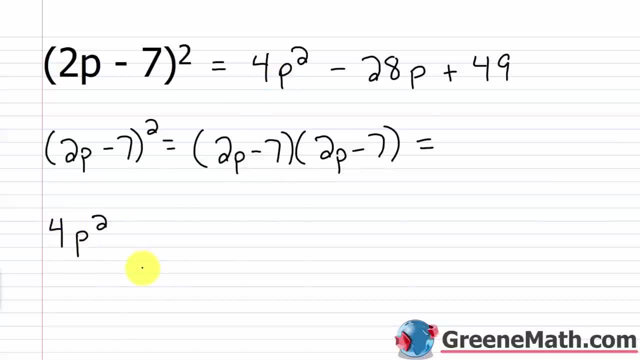 Exactly what we have here. Then the next thing we'd have is the outer terms: Two p times negative seven, that's minus 14 p. And we'd have your inner terms: Negative seven times two p, that's minus 14 p. Then the last terms: Negative seven times negative seven is plus 49.. When we combine like: 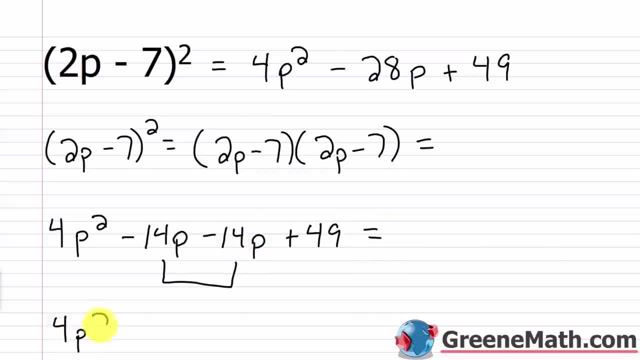 terms. here we're going to end up with four p squared minus 28 p plus 49, which again is exactly what we got by using our shortcut. All right, let's take a look at another one. We have six k plus one. This quantity is squared. 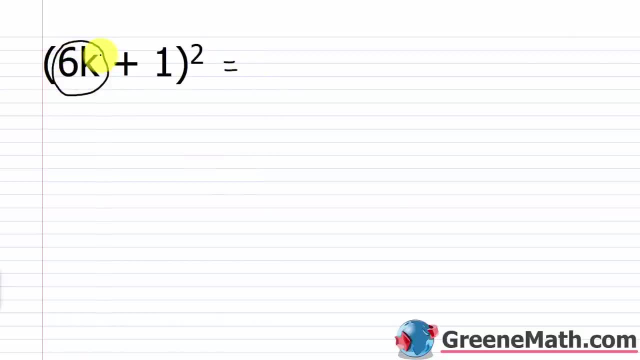 So again, what I want to do is take the first term. In this case that's six k, and I want to square it. So don't just write six k squared Again, I'm squaring that whole thing. So if I 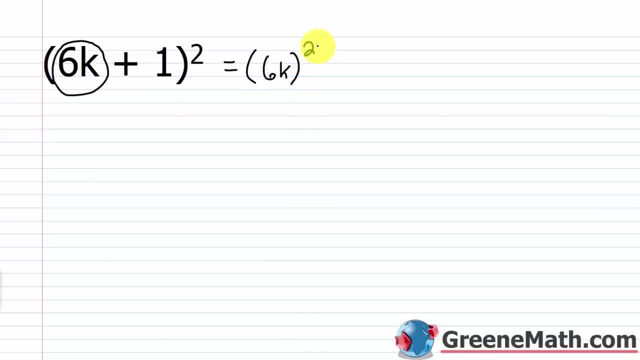 square the whole thing. you know, a good practice is just put everything in parentheses- the six and the k- and square it. That way you know that the six is squared and so is the k. So six squared is 36.. And k squared is k squared. Okay, then, plus we have two times whatever's in this position. 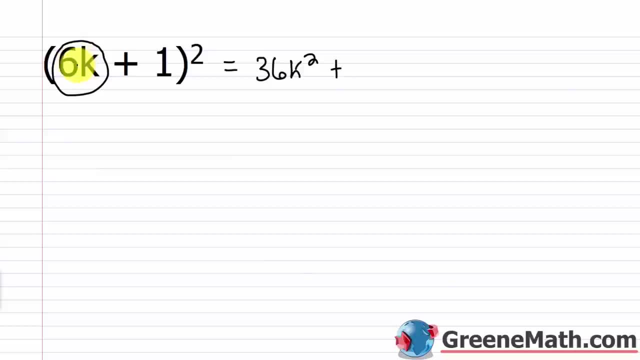 which is six k. Two times six is 12.. Times k is just 12 k. And then times whatever's in this position, which is one, So one times anything is itself. So this is just 12 k. And then lastly, 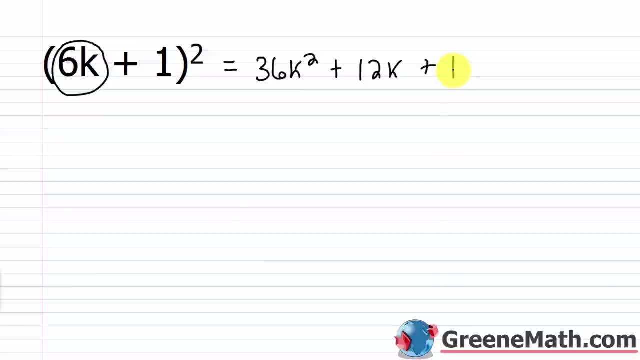 plus whatever's in this position squared, So one squared is just one. So we get 36 k squared plus 12 k plus one. And again we can prove this- We have six k plus one squared. So this is six k plus one times six k plus one. 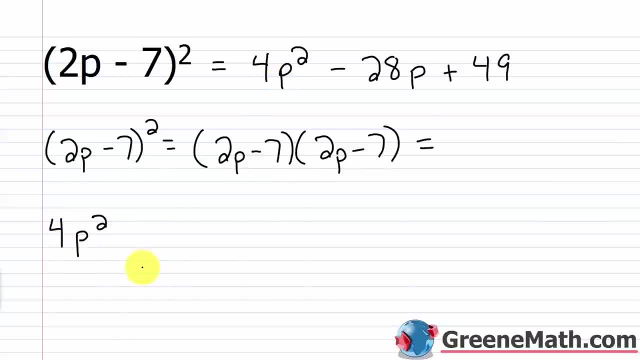 Exactly what we have here. Then the next thing we'd have is the outer terms. 2p times negative 7, that's minus 14p. Then we'd have your inner terms. Negative 7 times 2p, that's minus 14p. Then the last terms. Negative 7 times negative 7 is plus 49. 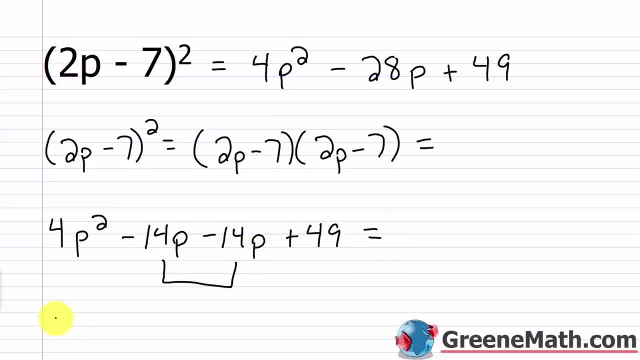 When we combine like terms here, we're going to end up with 4p squared minus 28p plus 49, which again is exactly what we got by using our shortcut. 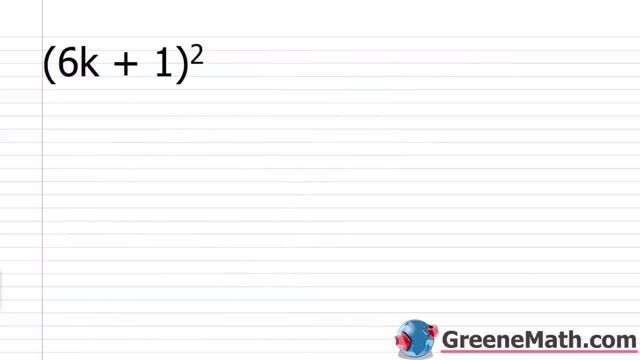 Alright, let's take a look at another one. We have 6k plus 1. This quantity is squared. 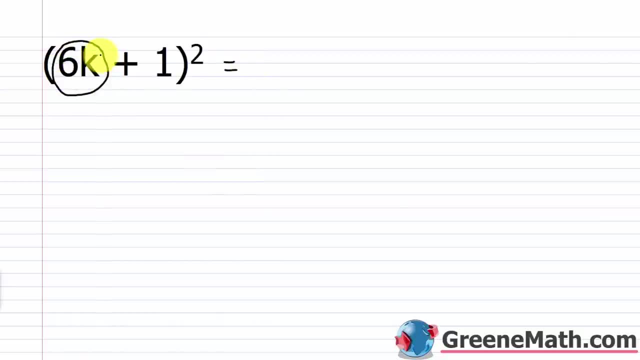 So again, what I want to do is take the first term, in this case that's 6k, and I want to square it. So don't just write 6k squared. Again, I'm squaring that whole thing. So if I square the whole thing, you know a good practice is to just put everything in parentheses, the 6 and the k, and square it. 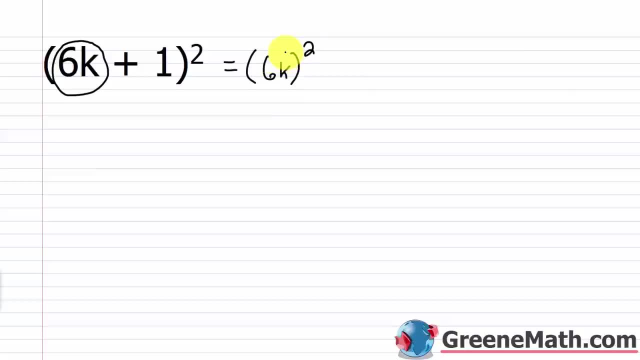 That way you know that the 6 is squared, and the k is the same. So 6 squared is 36, and k squared 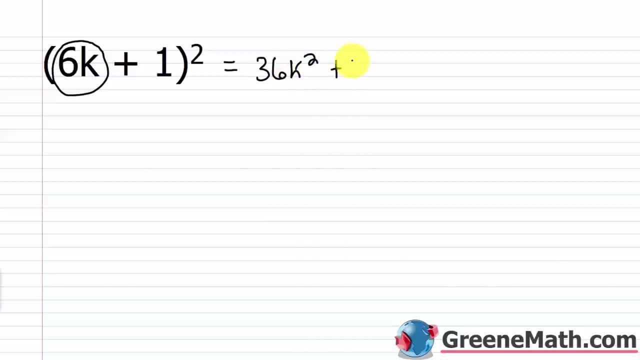 is k squared. Okay, then plus, we have 2 times whatever's in this position, which is 6k. 2 times 6 is 12, times k is just 12k, and then times whatever's in this position, which is 1. 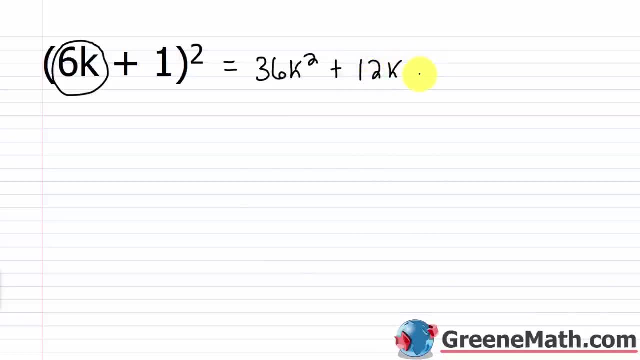 So 1 times anything is itself, so this is just 12k. Lastly, plus whatever's in 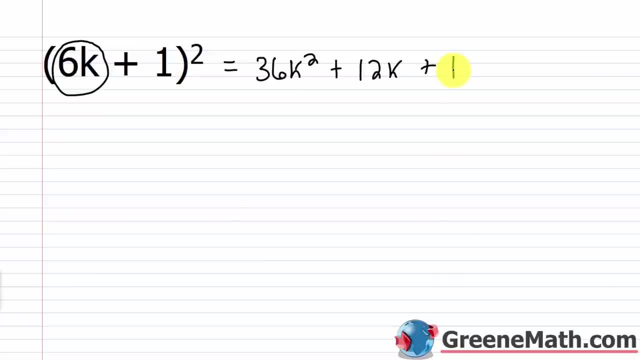 this position squared. So 1 squared is just 1. So we get 36k squared, plus 12k, plus 1. And again, we can 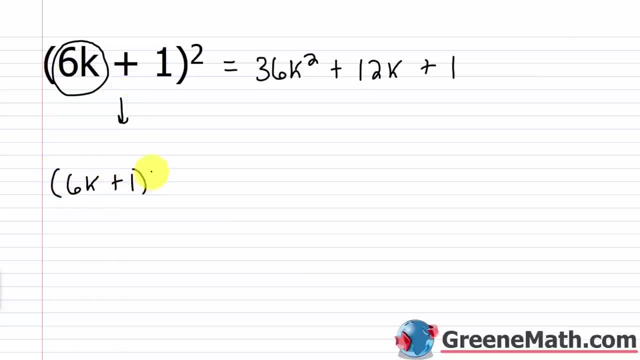 prove this. We have 6k plus 1 squared. 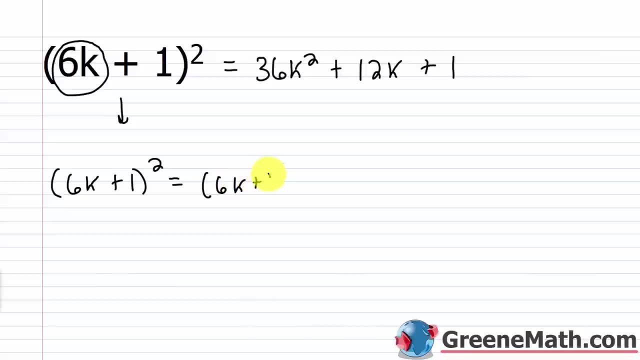 So this is 6k plus 1 times 6k plus 1. 6k times 6k is 36k squared. 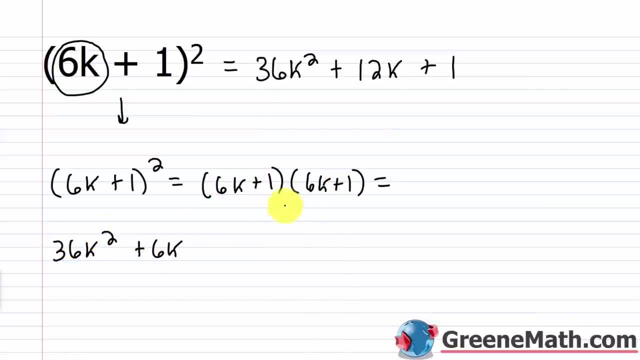 6k times 1 is plus 6k. 1 times 6k is again, plus 6k. And lastly, 1 times 1 is 1. 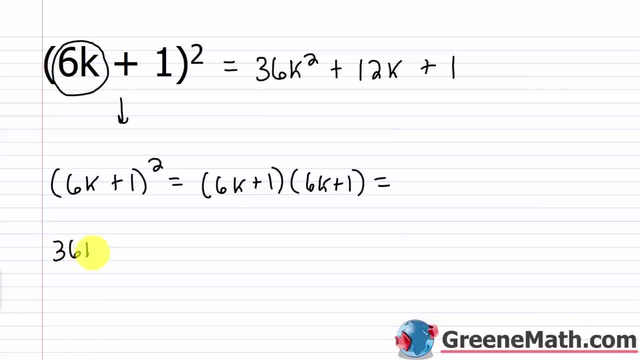 Six k times six k is 36 k. squared, Six k times one is plus six k. One times six k is again plus six k, And then, lastly, one times one is one. So we get 36 k squared plus six k plus six k is 12.. 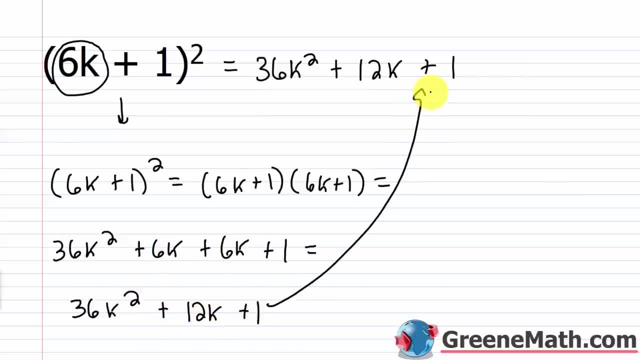 Okay, plus one. Again, exactly what you got there by using the shortcut. Let's take a look at 3x plus 2y squared, And again, all I'm going to do is whatever I have in the first position, I'm going. 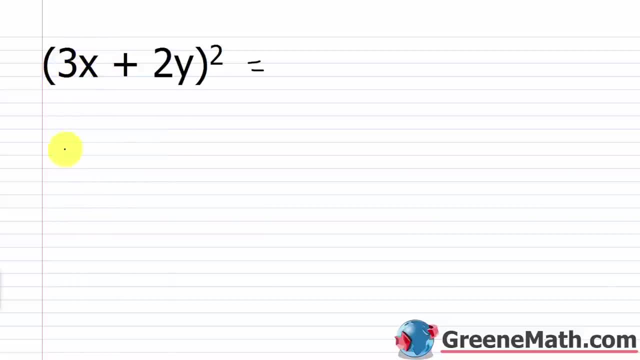 to square that. So the three has to be squared, and so does the x. Again, this is 3x. That term is squared, The whole thing. Please don't just write 3x squared, That's wrong. So three squared. 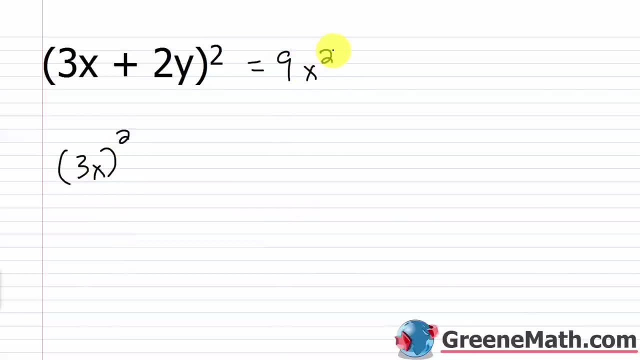 is nine and x squared is x squared, Then the next thing I want to do is have plus two times the first term times the second term. So two times three is six, Six times two is 12.. So plus 12.. Then, of course, the 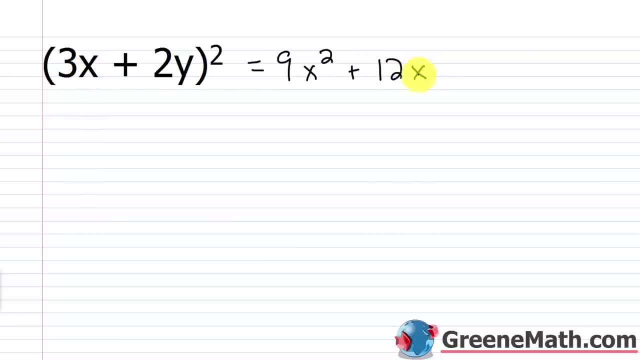 variables just come along for the ride. So x times y, So 12xy. Then lastly I have the final term, which is 2y squared. Again, I got to square the whole thing. Whole thing is squared. So two squared is four, Y squared is just y squared, right? Please again don't. 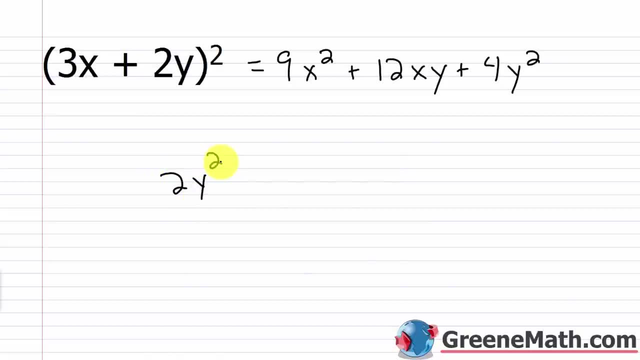 just write 2y squared. A lot of students they try to do this as fast as they can and they make a little small errors like that. This formula is only good if you practice it correctly, right? If you don't do it correctly, you might as well just go through and do it the long way. So we're. 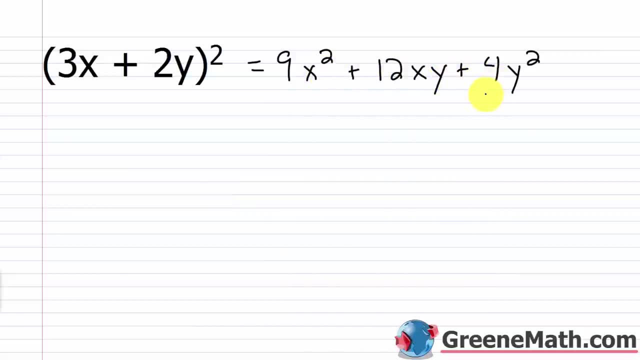 going to end up with 9x squared plus 12xy plus 4y squared, And again, let me do this the long way and prove this to you. So if I expand this, I get 3x plus 2y times 3x plus. 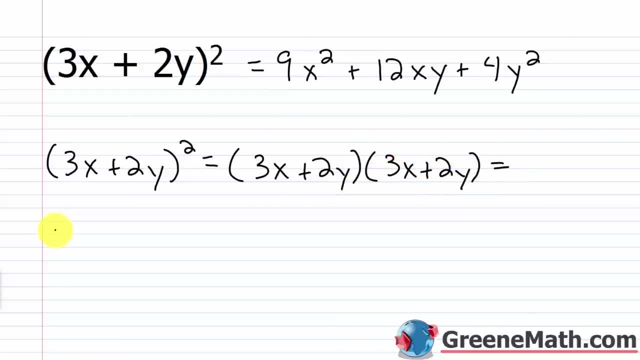 2y 3x times 3x is 9x squared. 3x times 2y is going to be plus 6xy, And then 2y times 3x again is plus 6xy, And then finally, plus 2y times 2y is 4y squared. So if I combine, 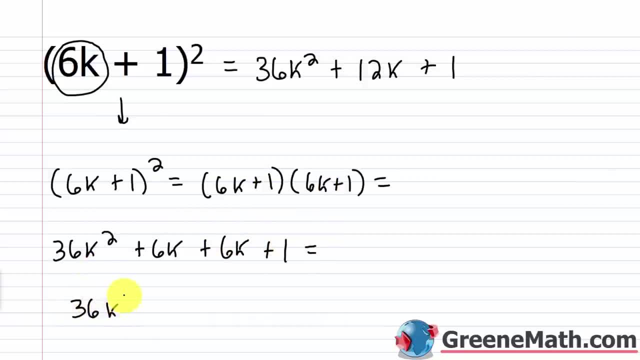 So we get 36k squared, plus 6k plus 6k is 12k, plus 1. 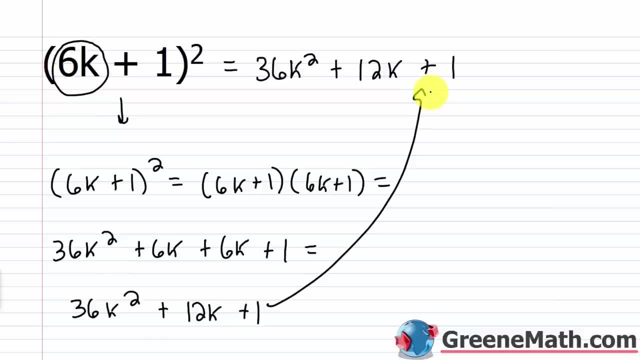 Again, exactly what you got there by using the shortcut. 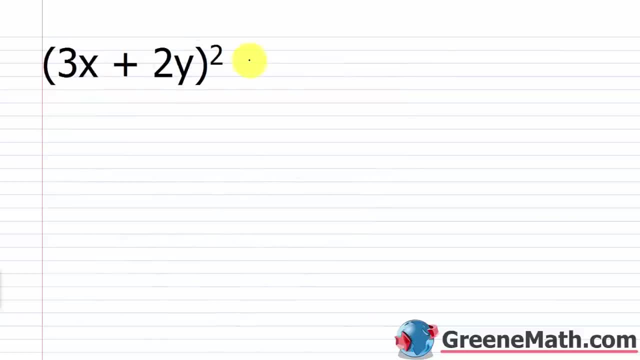 Let's take a look at 3x plus 2y squared. And again, all I'm going to do is, whatever I have in the first position, I'm going to square that. So the 3 has to be squared, and so does the x. Again, this is 3x. That term is squared. The whole thing. 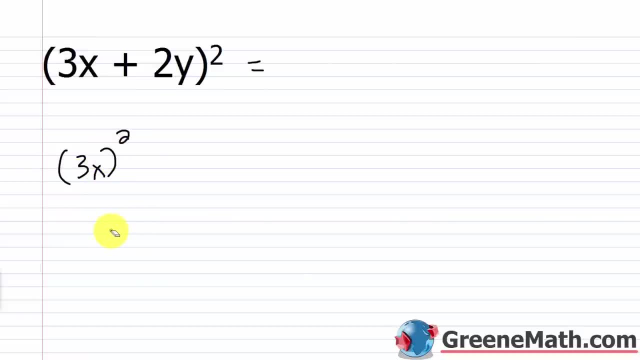 Please don't just write 3x squared. That's wrong. So 3 squared is not 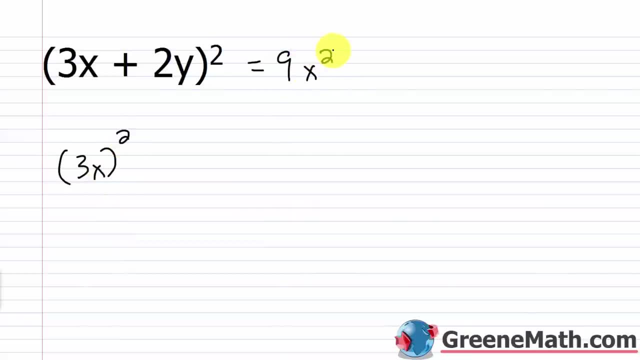 fine. And x squared is x squared. 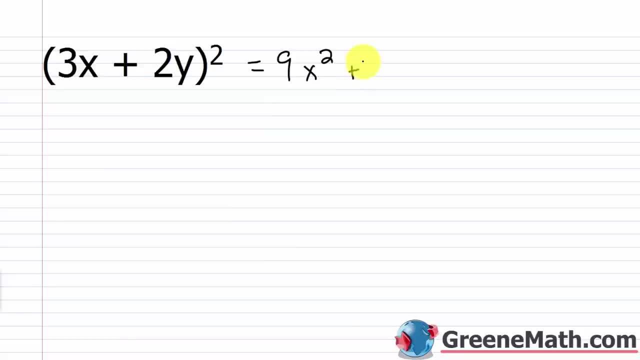 Then the next thing I want to do is have plus 2 times the first term times the second term. So 2 times 3 is 6. 6 times 2 is 12. So plus 12. 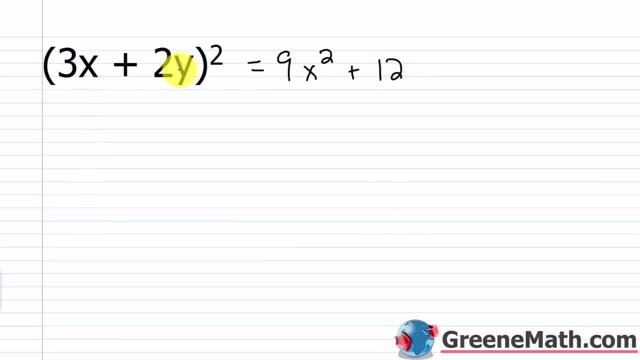 Then of course the variables just come along for the ride. So x times y. So 12xy. 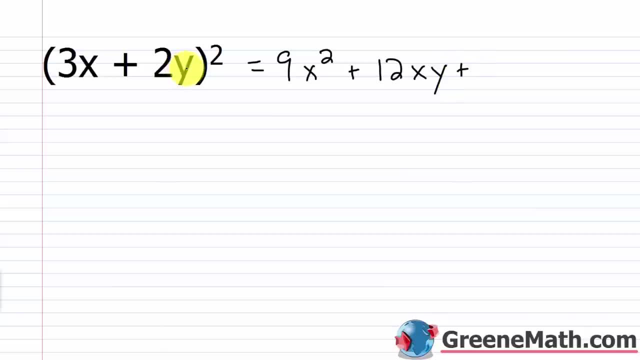 Then lastly I have the final term, which is 2y squared. 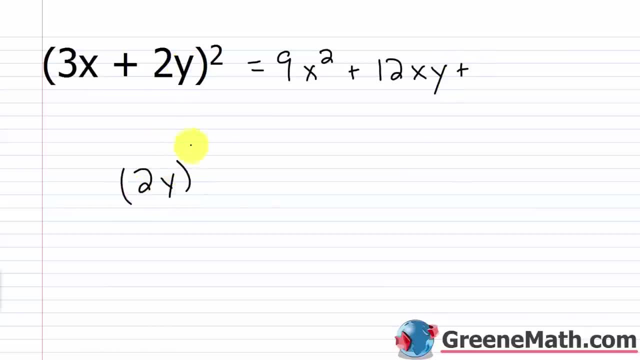 Again, I've got to square the whole thing. The whole thing is squared. 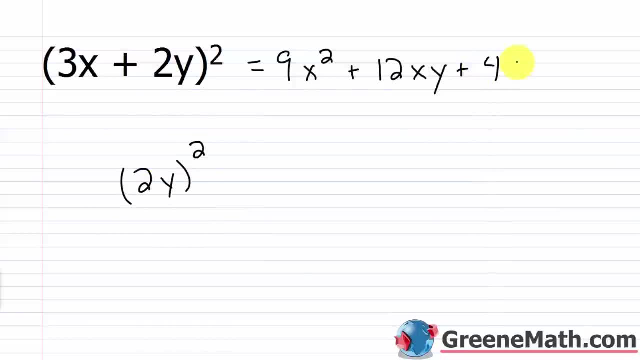 So 2 squared is 4. y squared is just y squared. 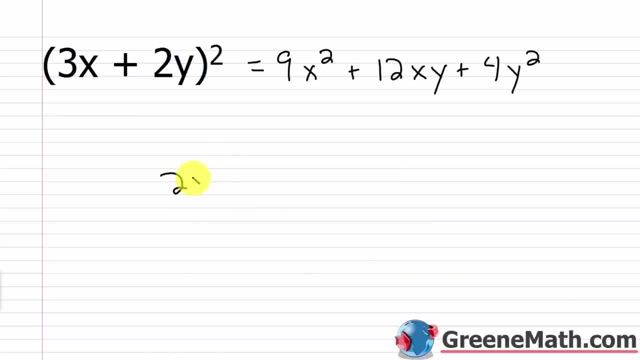 Please again, don't just write 2y squared. 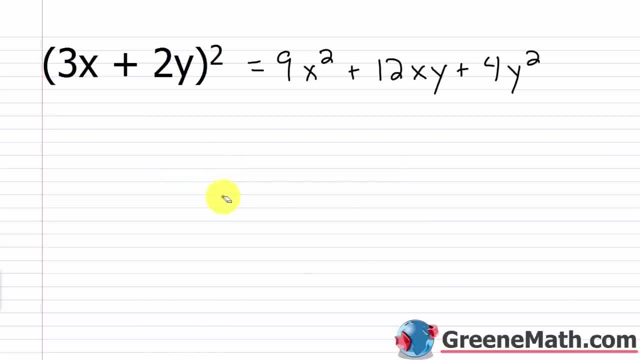 A lot of students, they try to do this as fast as they can, 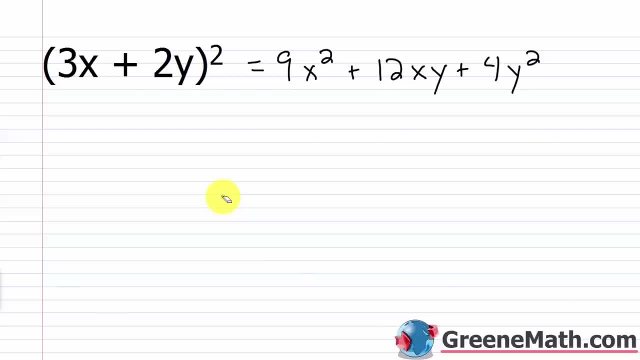 and they make little small errors like that. This formula is only good if you practice it correctly. 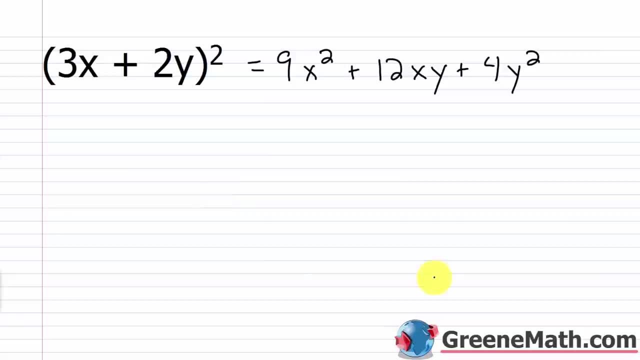 If you don't do it correctly, you might as well just go through and do it the long way. 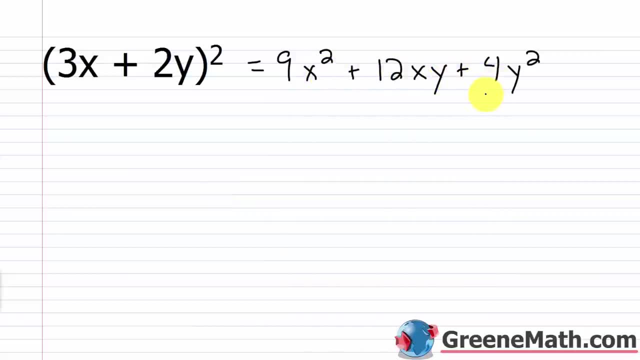 So we're going to end up with 9x squared plus 12xy plus 4y squared. 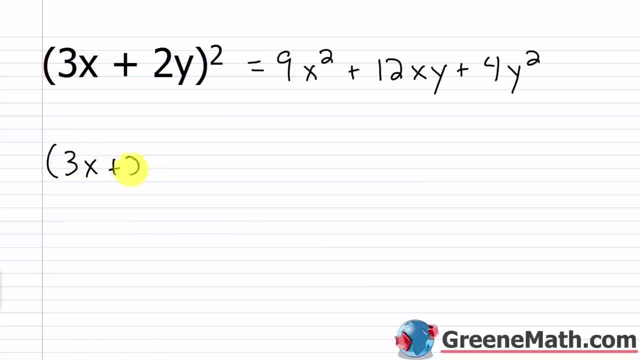 And again, let me do this the long way and prove this to you. 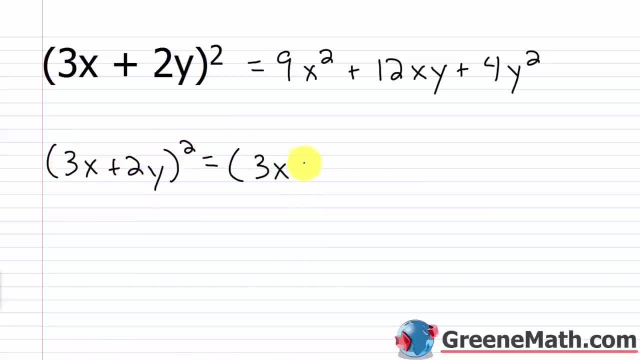 So if I expand this, I get 3x plus 2y times 3x plus 2y. 3x times 3x is 9x squared. 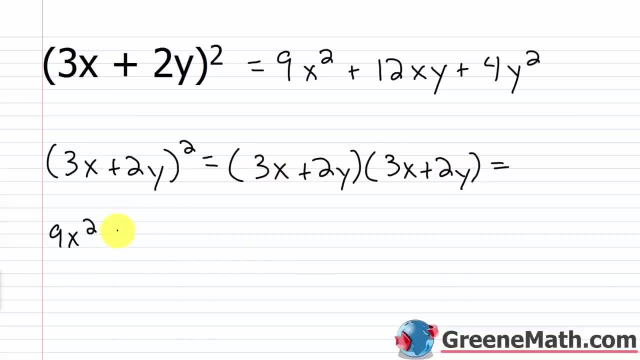 3x times 2y is going to be plus 6xy. 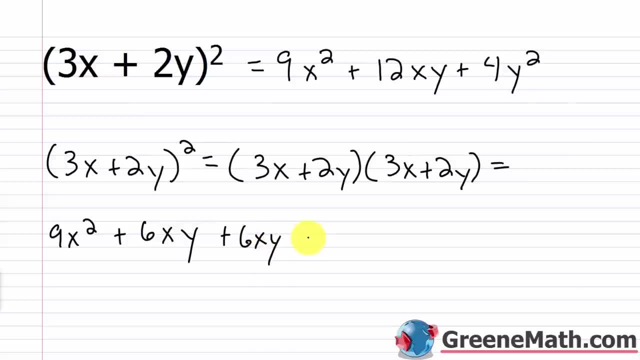 And then 2y times 3x again is plus 6xy. 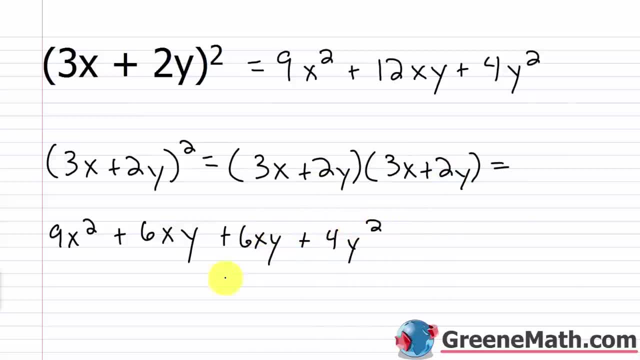 And then finally plus 2y times 2y is 4y squared. 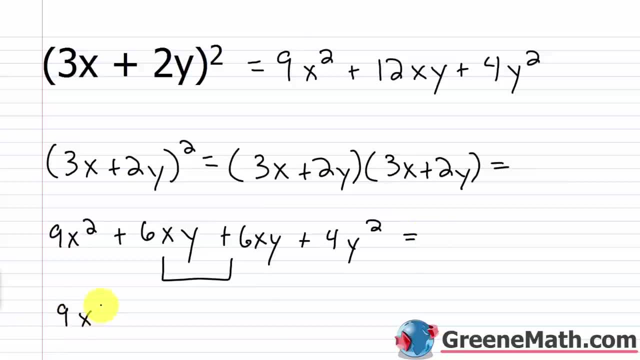 So if I combine like terms in the middle here, I get exactly what I got from my shortcut, which is 9x squared plus 12xy. Plus 4y squared. 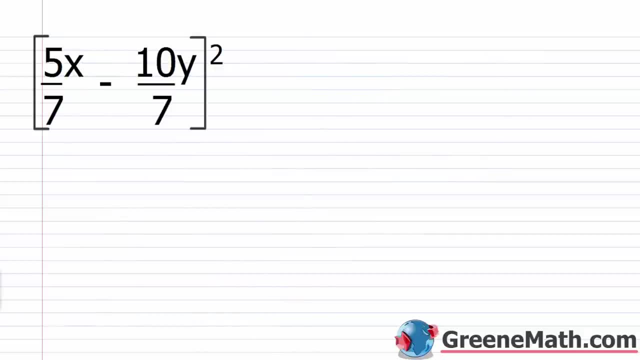 Let's look at one final problem here, and we're going to move on to some other common formulas. 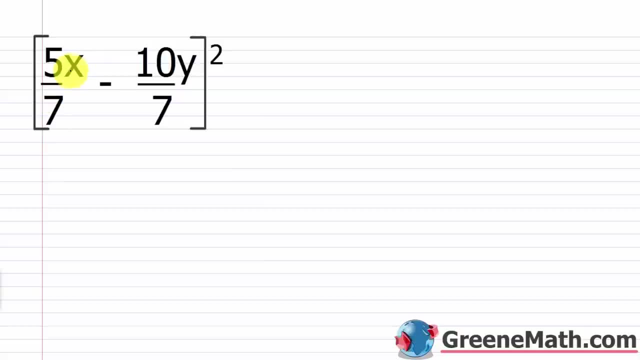 And we can use this with fractions as well. We have 5 sevenths x minus 10 sevenths y. 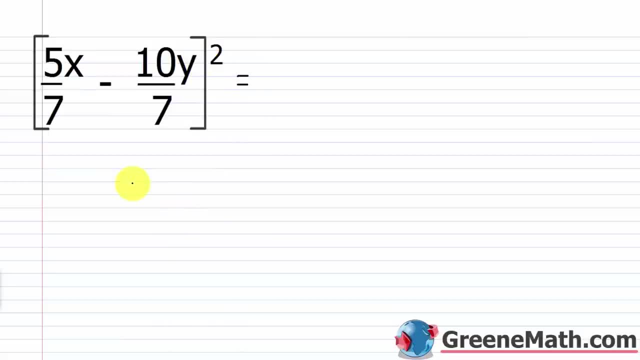 This quantity is squared. So again, I'm going to take whatever's in the first position, which in this case is 5 sevenths x, and I'm going to square it. 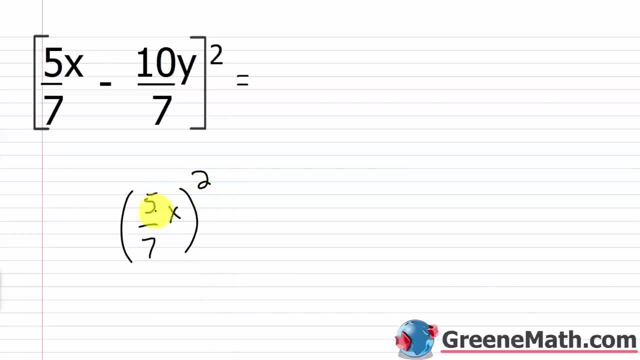 So to square this guy, if I square 5 sevenths, 5 times 5 is 25. 7 times 7 is 49. So that would be 25 forty-ninths. That's the square of 5 sevenths. And then we have x squared. 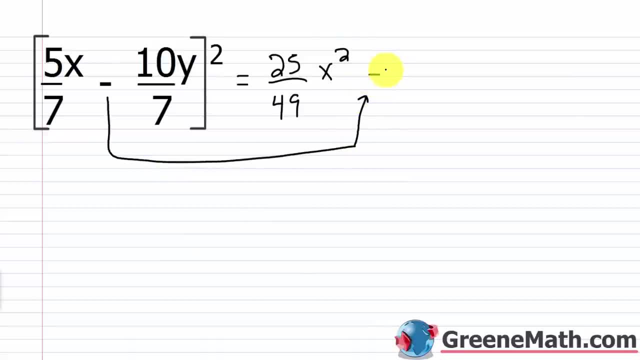 And remember, I have this minus here, so that's going to go right there. And next I'm going to have 2 times whatever's in this position, which is 5 sevenths, and then times x, I'm going to put these at the end for the variables, and then times 10 sevenths, whatever's in this position, and then times y. I'm trying to just see if there's anything I can cancel and there's not. 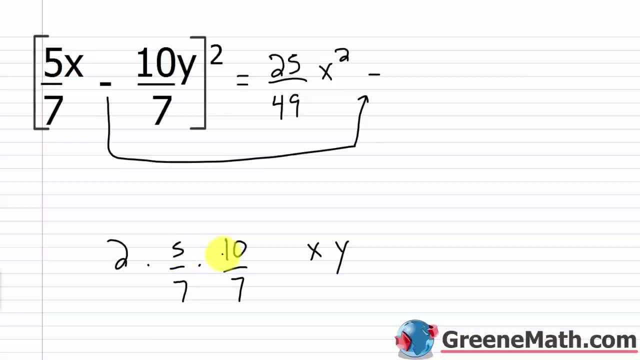 So you're going to have 2 times 5, which is 10. 10 times 10 is 100. So this is going to be 100 over 7 times 7, which is 49. And then times x, y. 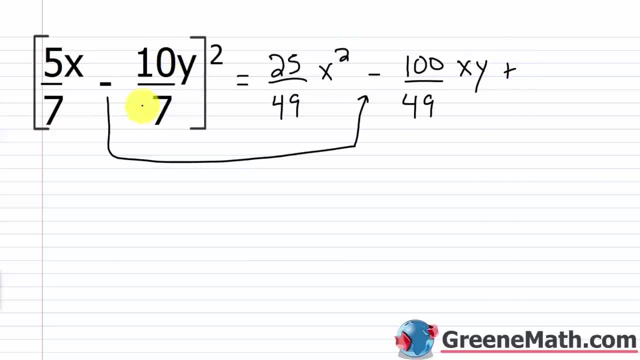 Alright, then lastly I'm going to have plus. This guy right here is squared. So 10 sevenths y. This is squared. So 10 squared is 100. 7 squared again is 49. 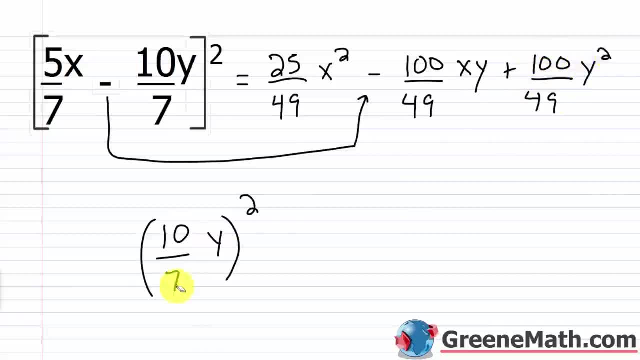 And y squared is of course just y squared. 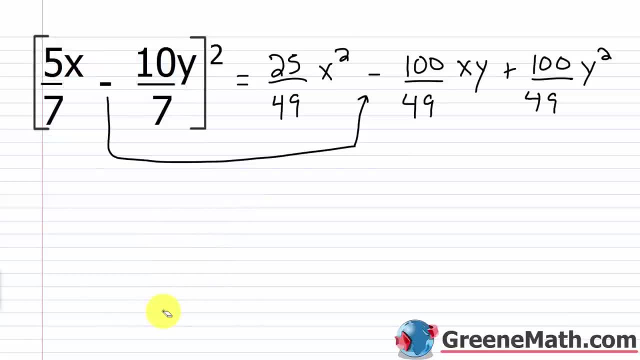 So there's your answer. You get 25 49ths x squared minus 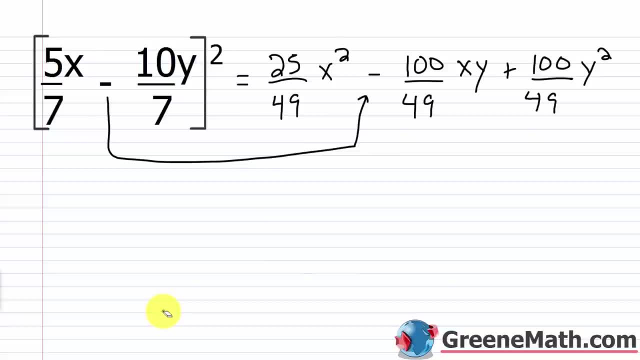 100 over 49 x y plus 100 over 49 y squared. 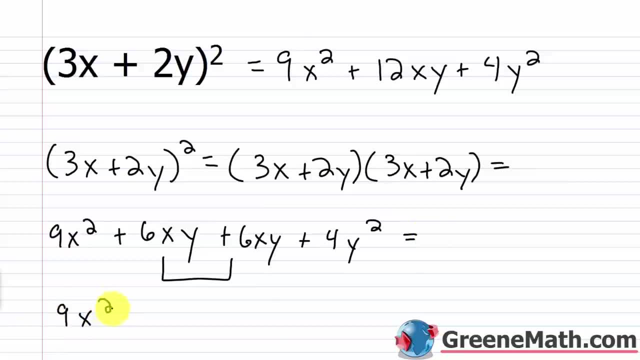 like terms in the middle. here I get exactly what I got from my shortcut, which is 9x squared plus 12xy plus 4y squared. One final problem here and we're going to move on to some other common formulas, And 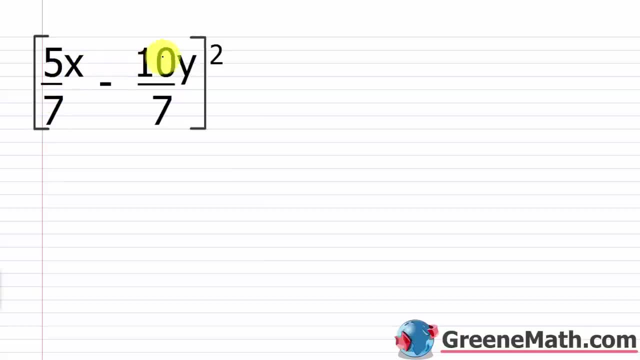 we can use this with fractions as well. We have 5 sevenths x minus 10 sevenths y. This quantity is squared. So, again, I'm going to take whatever's in the first position, which in this case is 5 sevenths x, and I'm going to square it. So, to square this guy, if I 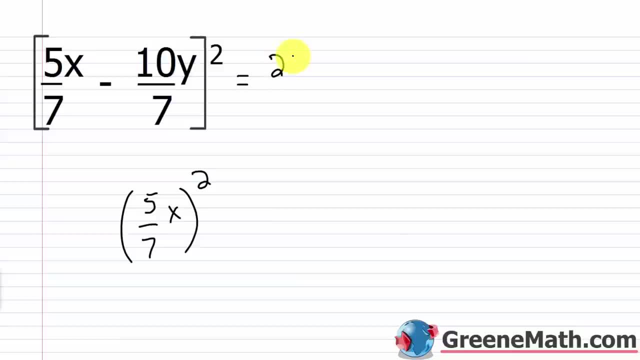 square 5 sevenths. 5 times 5 is 25.. 7 times 7 is 49.. So that would be 25 forty-ninths. That's the square of 5 sevenths. And then we have x squared. And remember, I have this: 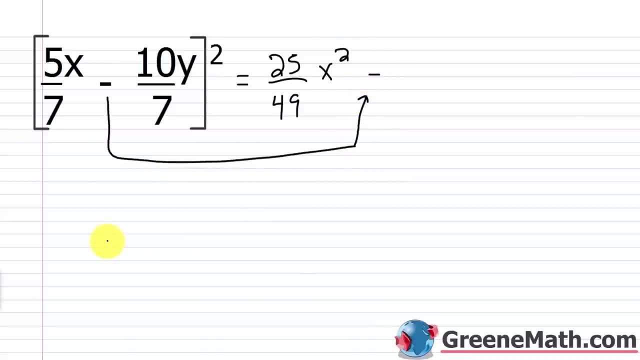 minus here. so that's going to go right there. And next I'm going to have 2 times whatever's in this position, which is 5 sevenths, and then times x- I'm going to put these at the end for the variables- and then times 10 sevenths, whatever's in this position, and then times. 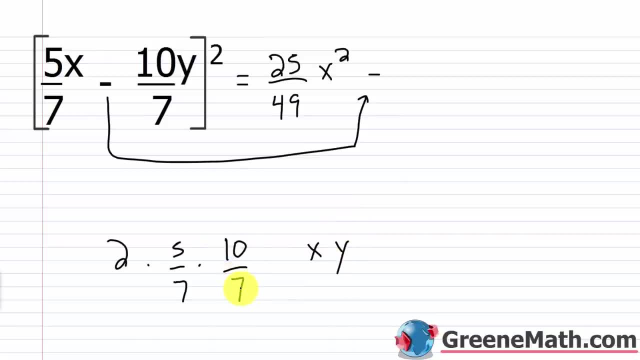 y, And I'm trying to just see if there's anything I can cancel, and there's not. So you're going to have 2 times 5, which is 10 sevenths, And then you're going to have 2 times 5, which. 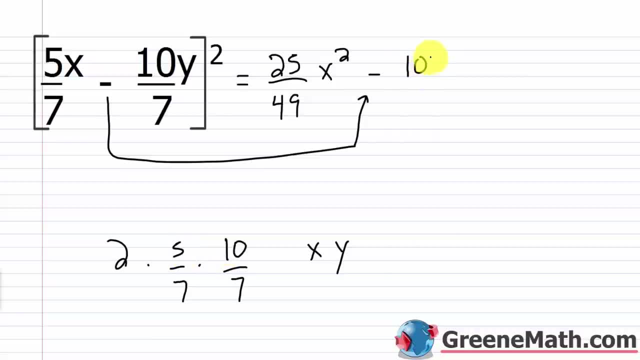 is 10.. 10 times 10 is 100.. So this is going to be 100 over 7 times 7,, which is 49, and then times xy. All right, Then, lastly, I'm going to have plus, This guy right here is squared, So 10. 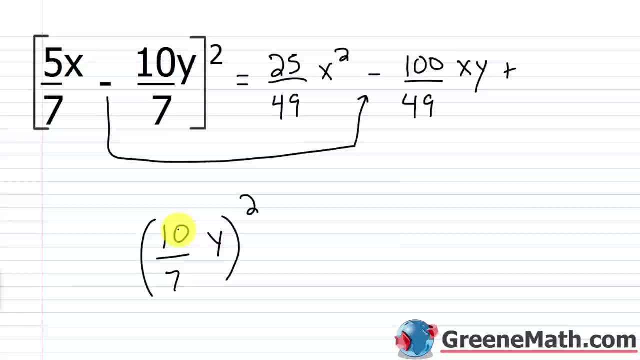 sevenths y. This is squared. So 10 squared is 100.. 7 squared again is 49.. And y squared is of course just y squared. So there's your answer. You get 25 forty-ninths And 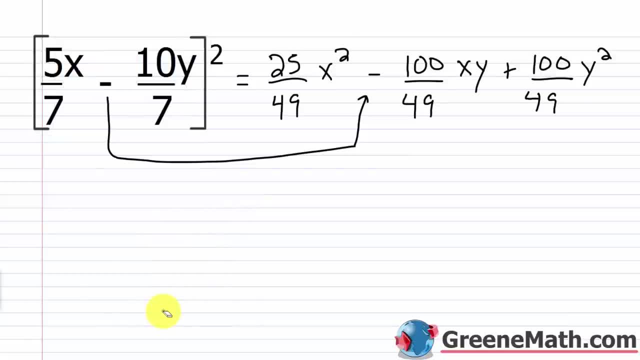 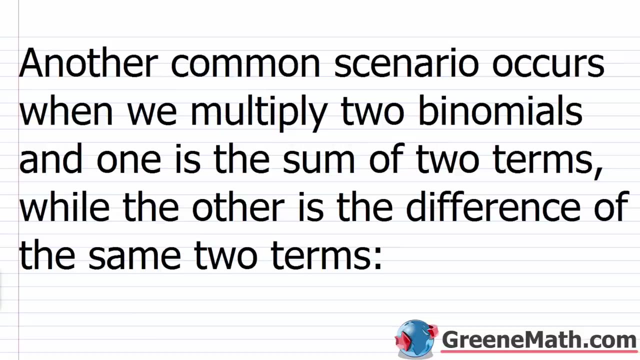 then if you take this guy and you expand it out, you can use FOIL, and you'll see that you get exactly this as your answer. All right, So let's move on now and talk about something else. So another common scenario. 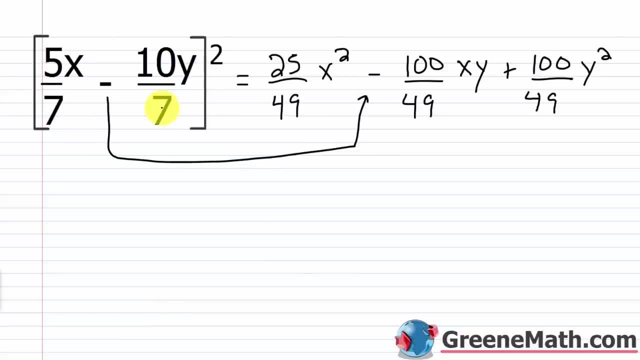 And again, if you want to, you can take this guy and you can expand it out, use FOIL, and you'll see that you get exactly this as your answer. 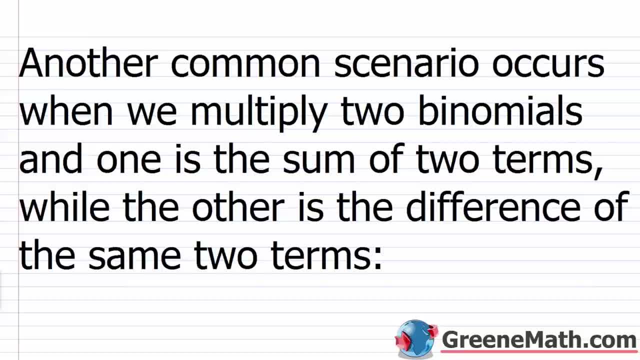 Alright, so let's move on now and talk about something else. 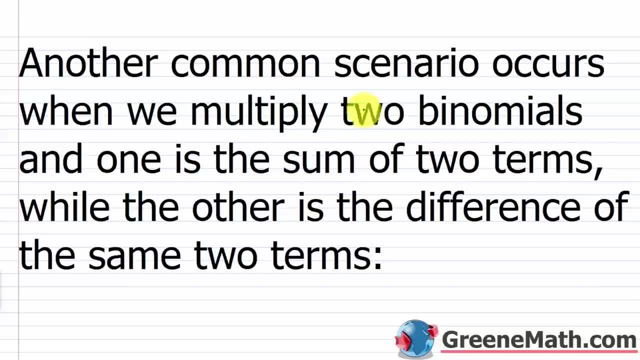 So another common scenario occurs when we multiply two binomials and one is the sum of two terms, while the other is the difference of the same two terms. 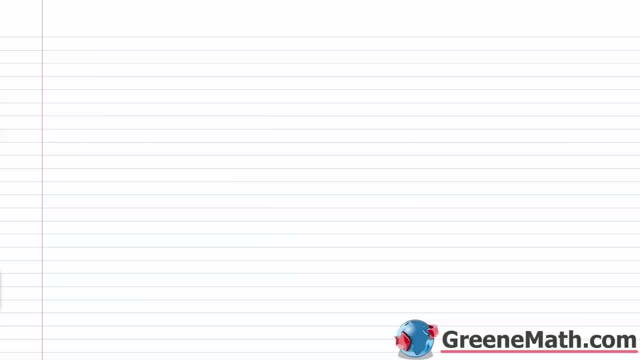 Now, the result of this we're going to learn later on is called the difference of two squares. Once you start talking about things like this, you're going to know what that means. So the difference of 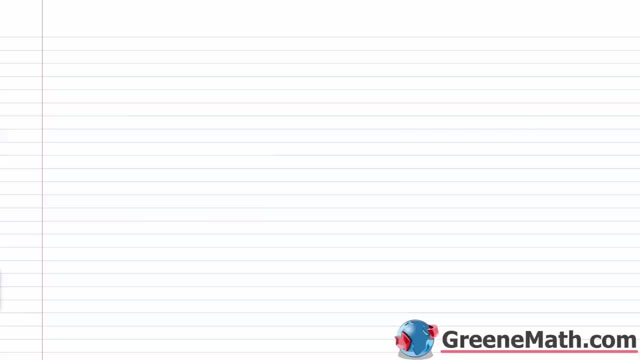 two squares is something you're going to come across all the time. Kind of once you hit it in factoring, moving forward, you're just going to keep talking about it over and over and over again. 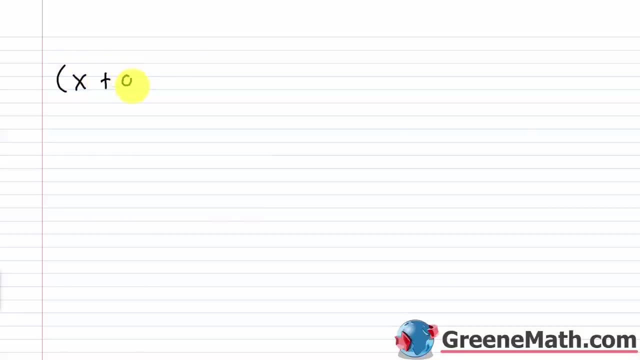 So it kind of looks like this. You have x plus, let's say, a times x minus a. So the same terms are in the same position of each binomial. So I have an x in the first position here and an x in the first position here. I have an a in the second position here and then the second position here. 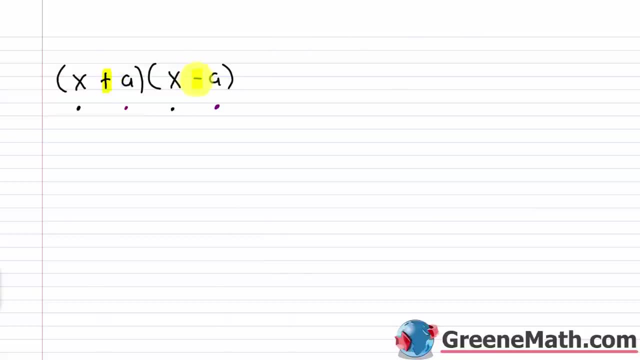 The only difference here is that I have a plus here and a minus here. So when you do this, what happens is the middle terms from the FOIL cancel themselves out. So let me show you that. So x times x is x squared. The outer terms, x times negative a is minus ax. The inner term, a times x is plus ax. So you can see those would cancel. And then a times negative a is minus a squared. So what 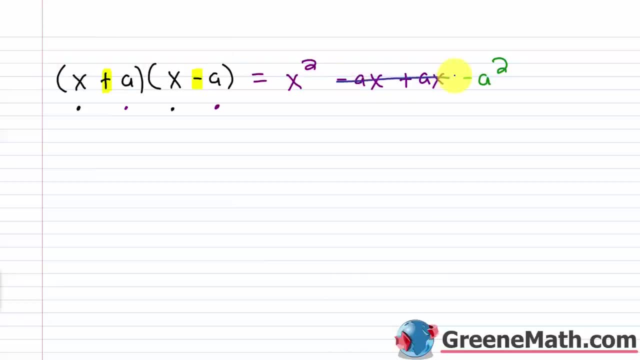 happens is the middle part is going to cancel itself out and you're left with x squared x squared minus a squared. 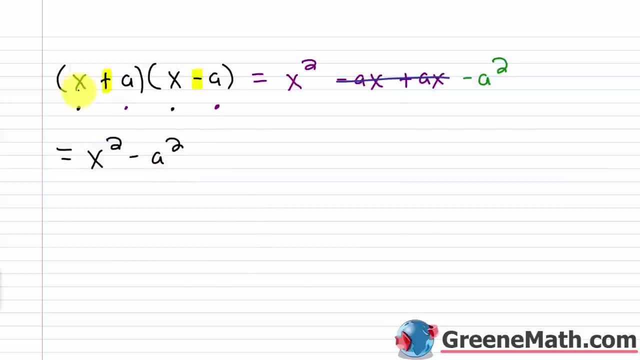 So in other words, the first term here is going to be squared minus the second term, which is squared. 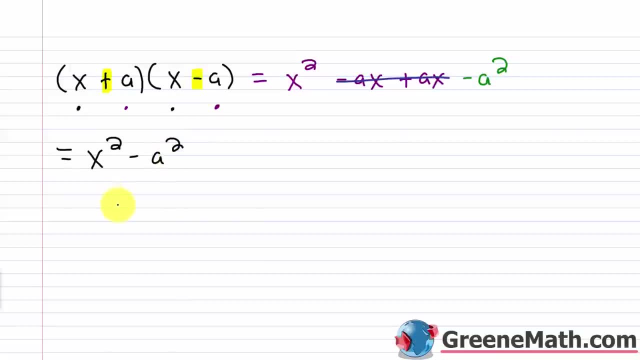 Whenever you come across this scenario. Again, this is referred to as the difference of two squares. Because you have subtraction involved, that's where difference comes in. And then each term is squared. So the difference of two squares. So here's kind of the generic formula that you probably see in your textbook. It's x plus y times x minus y. 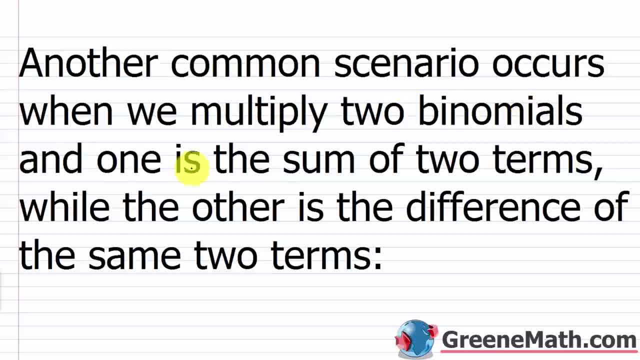 occurs when we multiply 2 binomials and one is the sum of two terms, while the other is the difference of the same term. So let's move on now to something else. So another common scenario occurs when we multiply 2 binomials, and one is the sum of two terms, while the other is the difference of the same term. 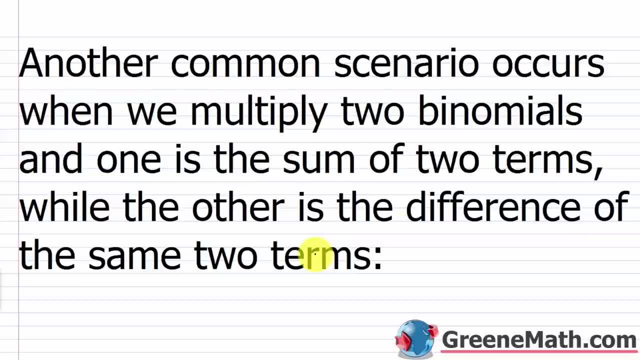 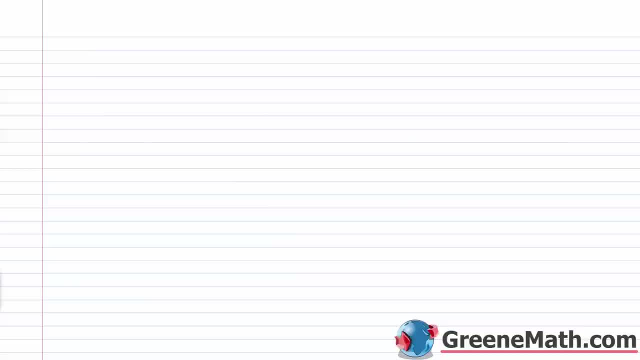 same two terms. Now, the result of this we're going to learn later on- is called the difference of two squares. Once you start talking about things like this, you're going to know what that means. So the difference of two squares is something you're going to come across all the time, Kind of once. 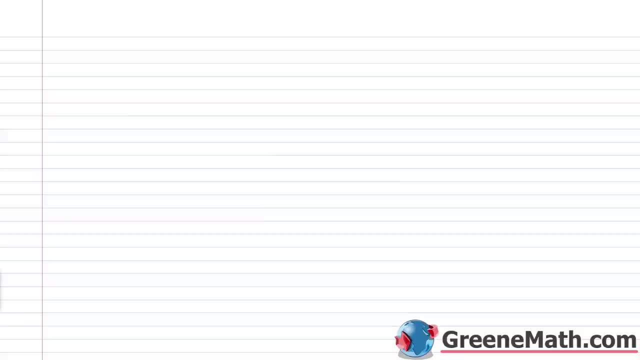 you hit it in factoring, moving forward. you're just going to keep talking about it over and over and over again. So it kind of looks like this: You have x plus, let's say, a times x minus a. So the same terms are in the same position of each binomial. So I have an x in the first position. 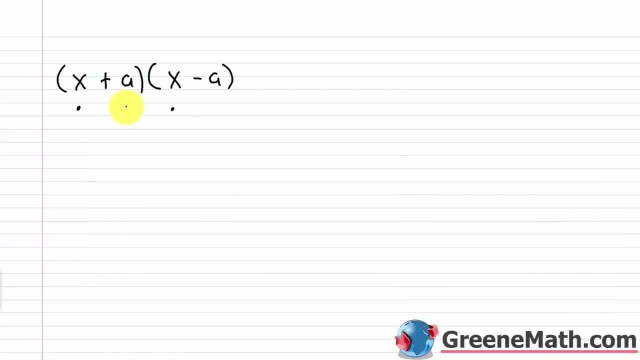 here and an x in the first position here. I have an a in the second position here and then the second position here. The only difference here is that I have a plus here and a minus here. So when you do this, what happens is the middle terms from the foil cancel themselves out. So let me show you. 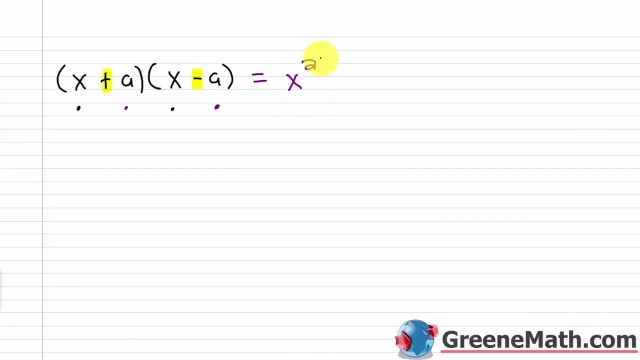 that. So x times x is x squared. The outer terms x times negative a is minus a x. The inner term a times x is plus a x. So you can see those would cancel. And then a times negative a is minus a squared. So what happens is the middle part is going to cancel. 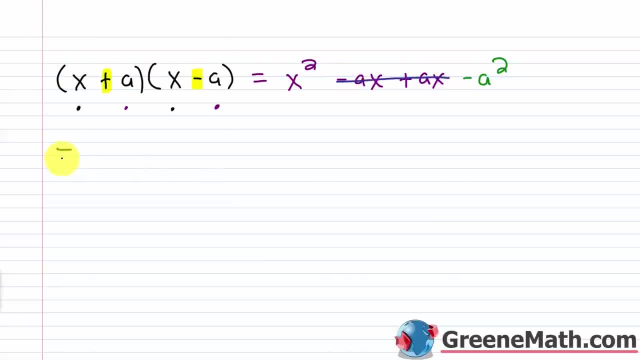 itself out and you're left with x squared, x squared minus a squared. So, in other words, the first term here is going to be squared minus the second term. So the first term here is going to be squared minus the second term, which is squared. Okay. whenever you come across this scenario, 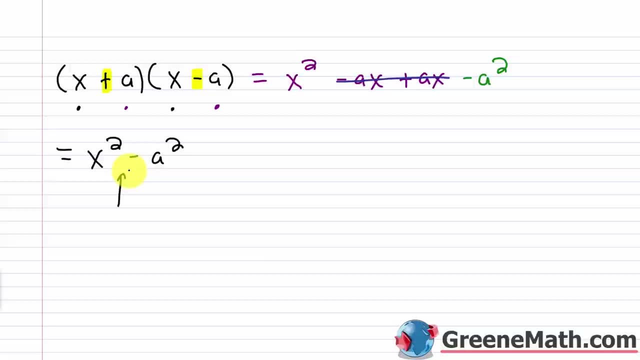 And again this is referred to as the difference of two squares. Right, because you have subtraction involved. that's where difference comes in, And then each term is squared. So the difference of two squares. So here's kind of the generic formula that you probably see in your textbook. Again, it's 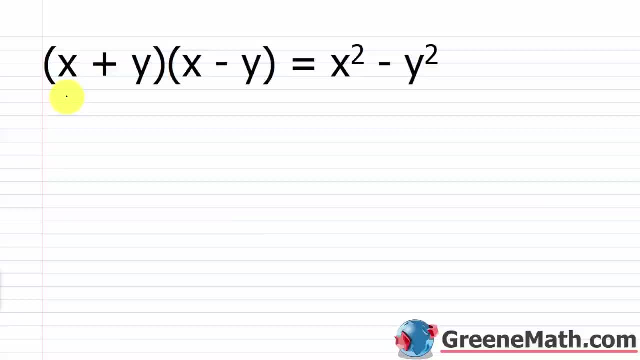 x plus y times x minus y. And again, the first position of each one is the same. I have x here and x here. The second position of each is the same. I have y here and y here. You've got to have that. You can't have something like you know: x plus three times x minus seven. That's not going. 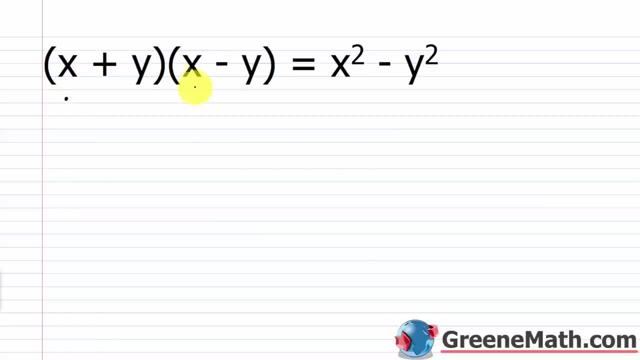 And again, the first position of each one is the same. I have x here and x here. The second position of each is the same. I have y here and y here. You've got to have that. You can't have something like x plus 3 times x minus 7. That's not going to work. You've got to have x plus 3 times x minus 3. 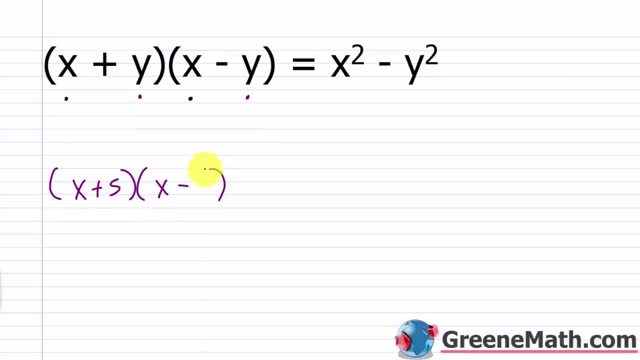 Or x plus 5 times x minus 5. 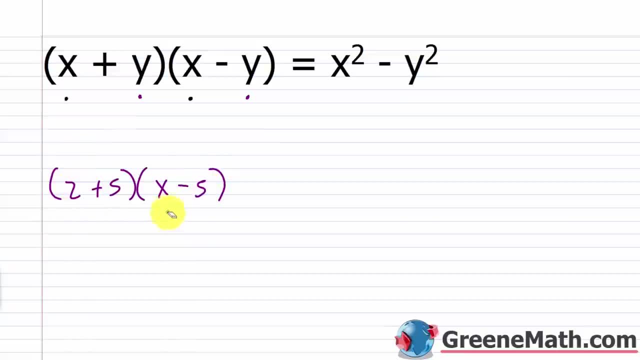 Or it could be z plus 5 times 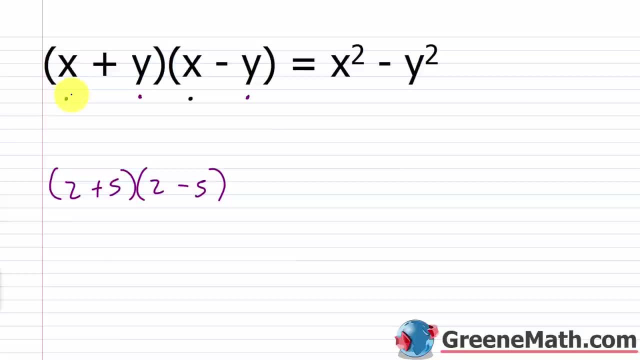 z minus 5. But the first term in the first binomial has to be the same 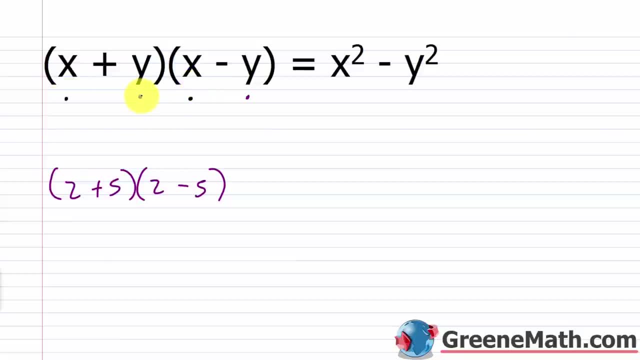 as the first term in the second binomial. The second term in the first binomial has to be the same as the second term in the second binomial. It has to be the same. 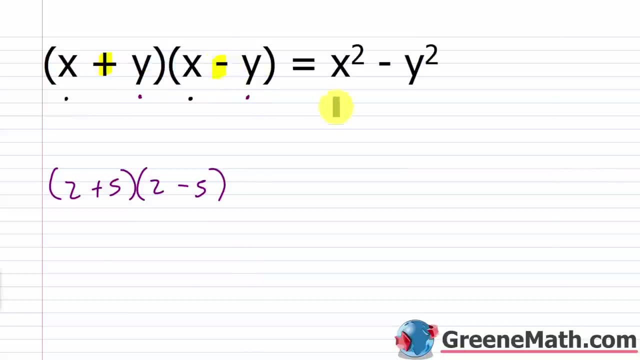 The only thing that's going to be different is the plus here and the minus here. 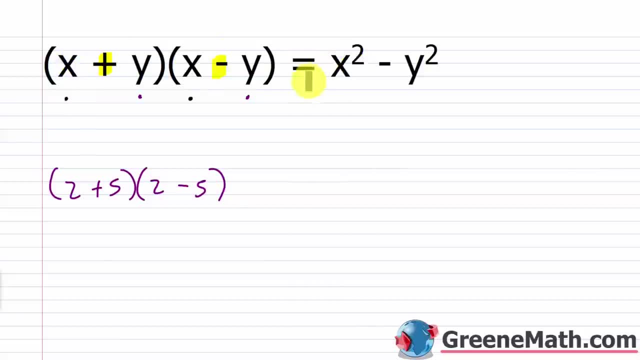 So you get this first term squared. So x is squared 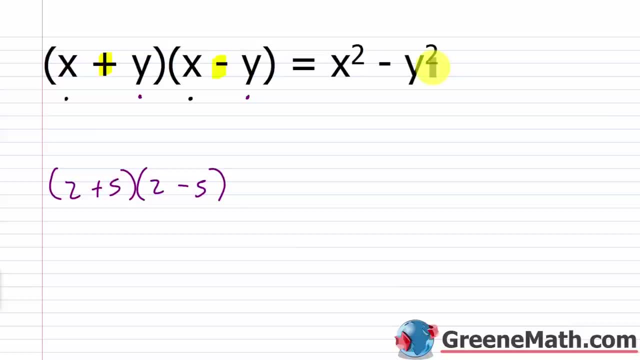 minus your second term squared. Remember, the middle terms are going to drop out when you do FOIL 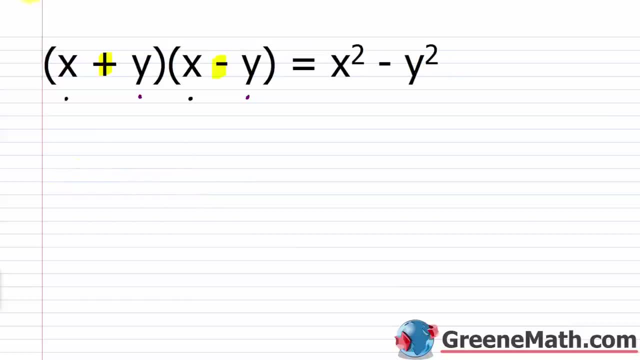 because they're opposites. So if I was to show you this one more time. 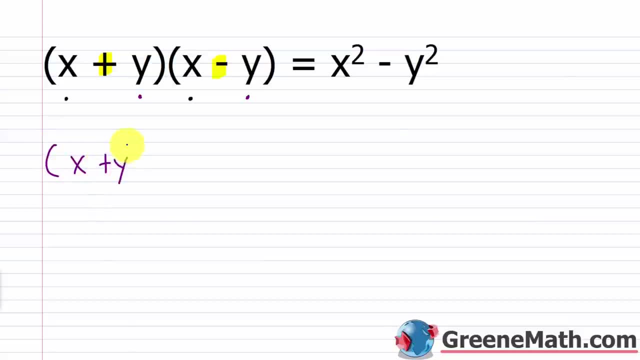 We have something like x plus y times x minus y. If we use FOIL, x times x is x squared. The outer x times negative y is negative xy. The inner y times x is plus xy. You see those are going to cancel. And then the last y times negative y is minus y squared. So this is going to go away in the middle here. That negative xy plus xy is going to cancel. 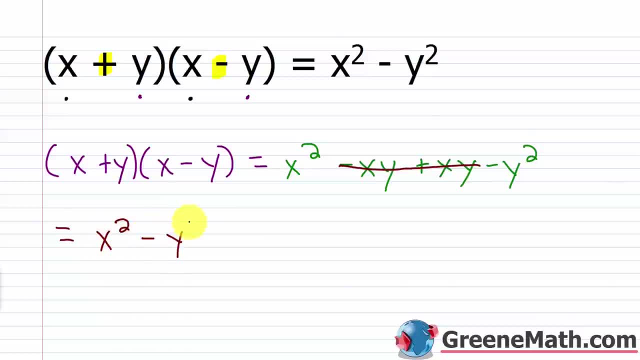 And what I'm left with is just x squared minus y squared. 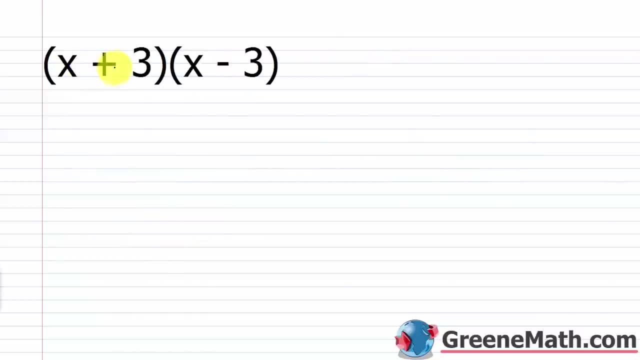 Alright, let's take a look at some examples. So I have x plus 3 times x minus 3. 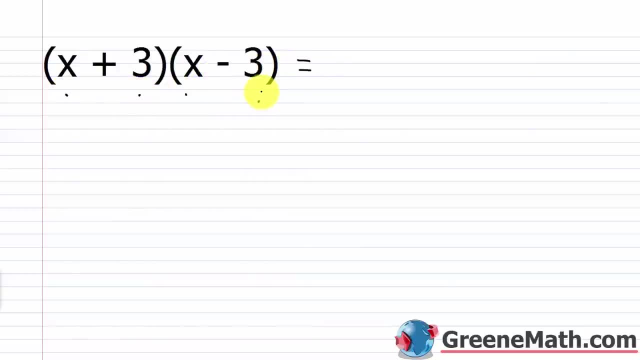 So again, same thing here and here. Same thing here and here. Here we go. So all I need to do is take the first term and square it and subtract away the second term and square it. 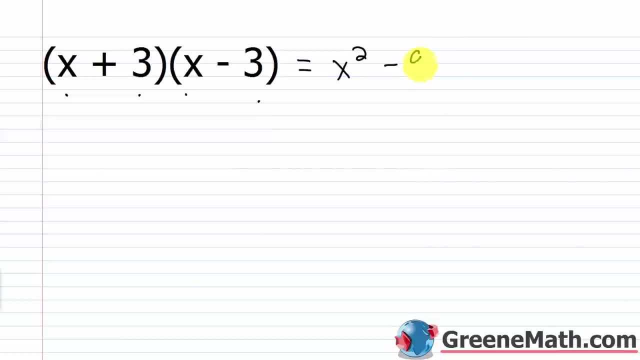 So 3 squared we know would be 9. So this ends up being x squared minus 9. 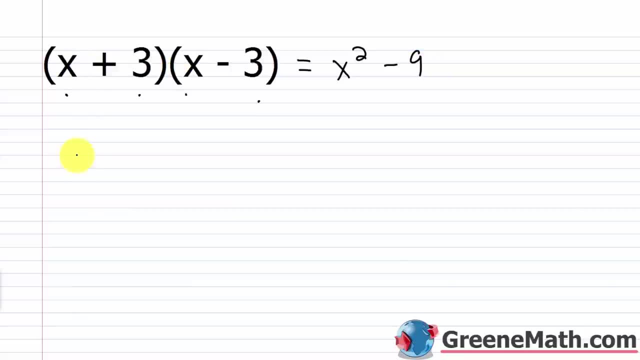 Again, you can verify this just by using FOIL. x times x is x squared. I'm going to kind of write this out 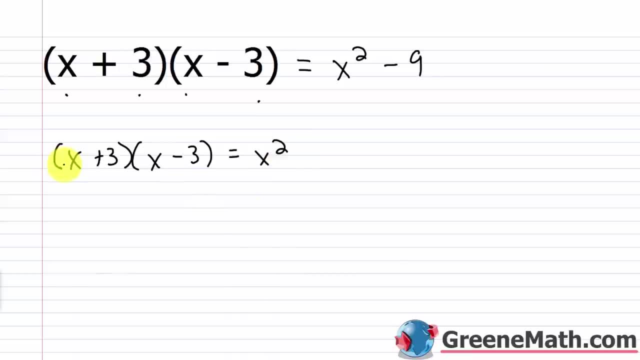 real quick. Then the outer x times negative 3 is minus 3x. 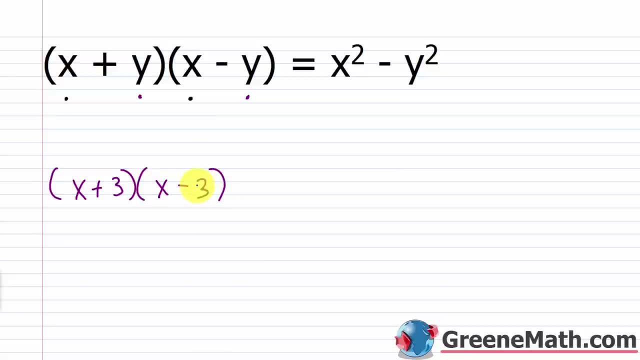 to work. You got to have x plus three times x minus three, Or x plus five times x minus five, Or it could be, you know, z plus five times z minus five. But the first term in the first binomial has to be the same as the first term in the second binomial. The second term in the 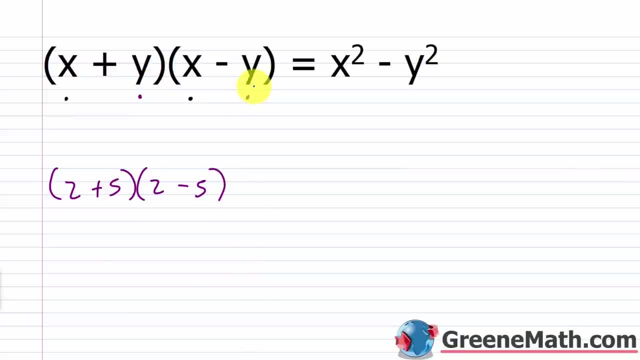 binomial has to be the same as the second term in the second binomial. The only thing that's going to be different is the plus here and the minus here. So you get this first term squared. so x is squared, minus your second term squared. 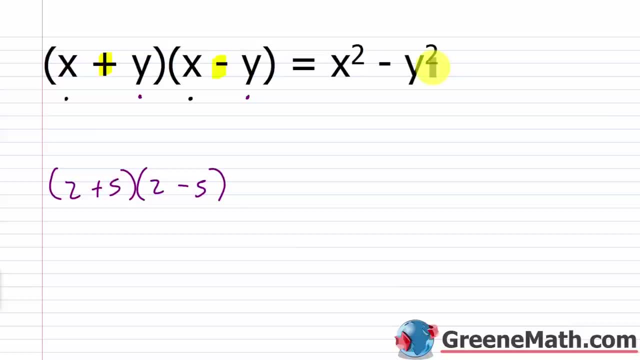 Remember, the middle terms are going to drop out when you do FOIL, because they're opposites. So if I was to show you this one more time, we have something like x plus y times x minus y. if we use FOIL, x times x is x squared, the outer x times negative, y is negative xy. 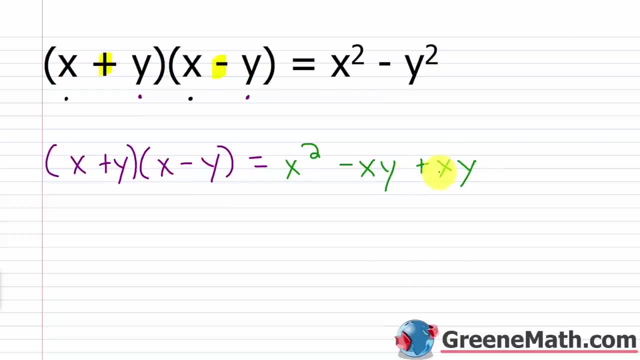 the inner y times, x is plus xy. you see, those are going to cancel. and then the last y times, negative y is minus y squared. So this is going to go away in the middle here. That negative xy plus xy is going to cancel and what I'm left with is just x squared minus. 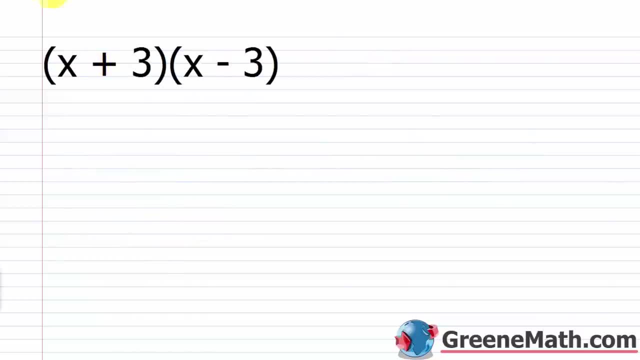 y squared. Alright, let's take a look at some examples. So I have x plus 3 times x minus y. So again, same thing here and here. same thing here and here. So I'm good to go. So all I need to do is take the first term and square it and subtract away the second. 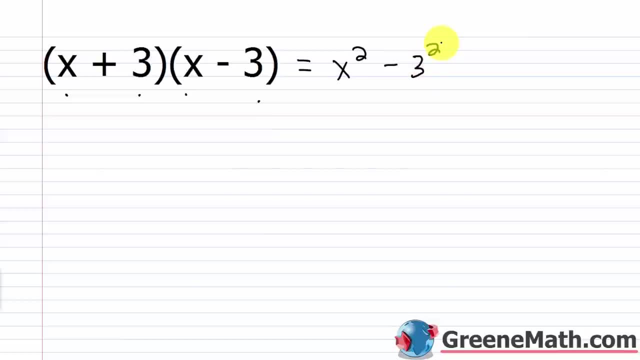 term and square it. So 3 squared, we know, would be 9.. So this ends up being x squared minus 9.. And again, you can verify this just by using FOIL: x times x is x squared. I'm going to kind of write this out real quick. 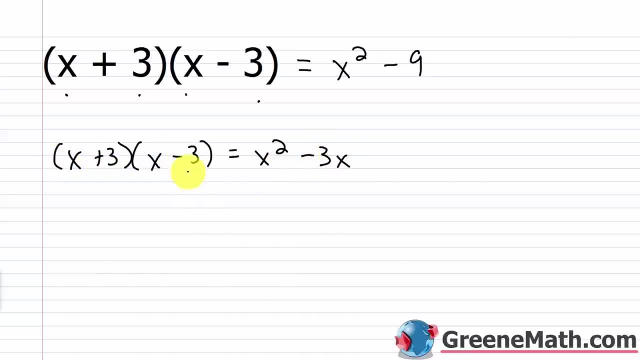 Then the outer x times negative 3 is x squared, This is minus 3x. The inner 3 times x is plus 3x, So those are going to cancel. and then the last 3 times negative, 3 is minus 9.. 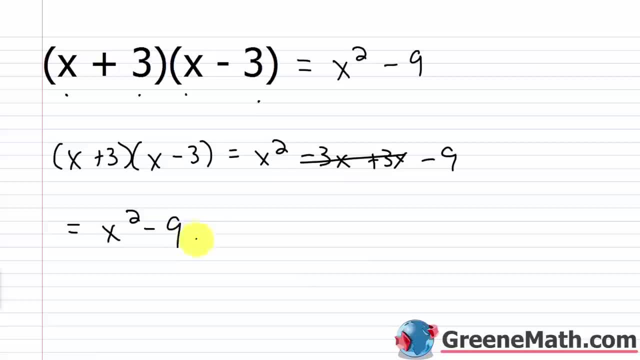 This cancels. Again, you end up with x squared minus 9.. So now we have 6x plus 1 times 6x minus 1.. So again, the first term is the same in each case. The second term is the same in each case. 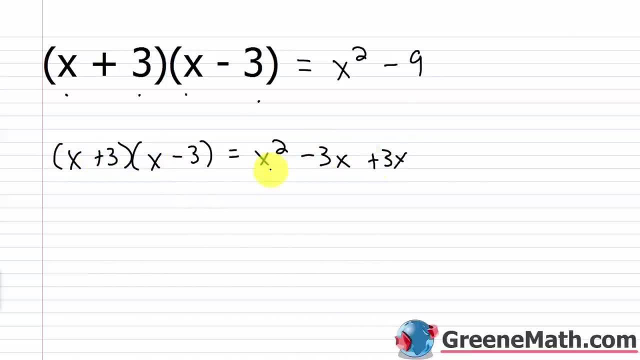 The inner 3 times x is plus 3x. So those are going to cancel. And then the last 3 times negative 3 is minus 9. This cancels. 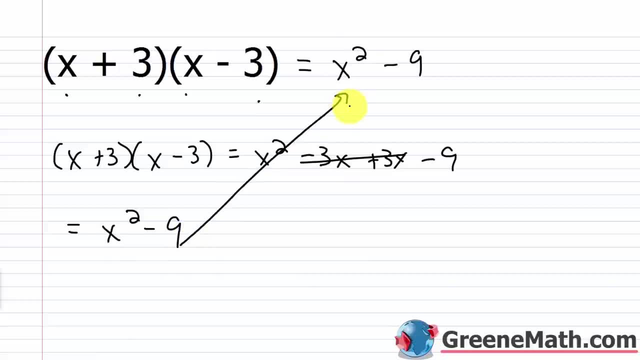 Again, you end up with x squared minus 9. 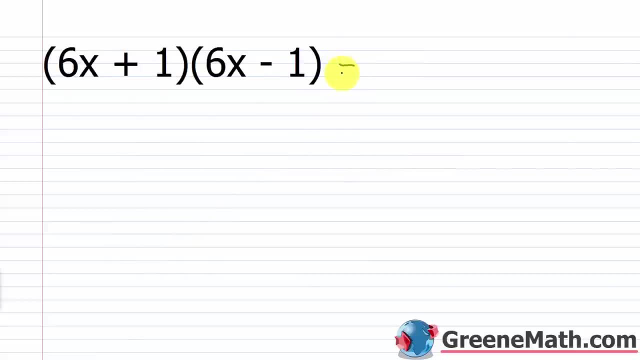 So now we have 6x plus 1 times 6x minus 1. So again, the first term is the same in each case. The second term is the same in each case. Just the plus and the minus is what's differing here. 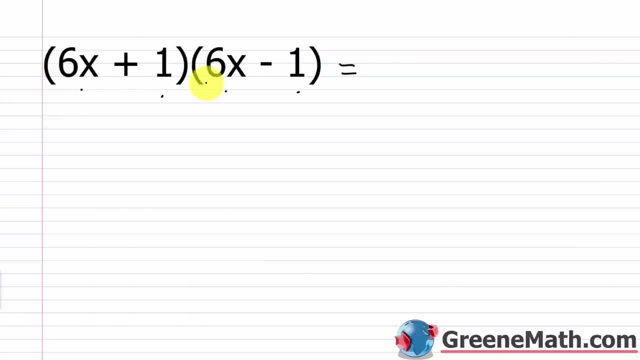 So then the first term is squared. Again, don't just write 6x squared and move on. Very, very common mistake. You've got to square the whole thing. The 6 and the x are both squared. 6 squared is 36. x squared is x squared. Then minus. I'm going to take that second term, which is 1, and I'm going to square that. We all know 1 squared is just 1. So this ends up being 36x squared minus 1. And again, go through and use FOIL and verify that I got the right answer. 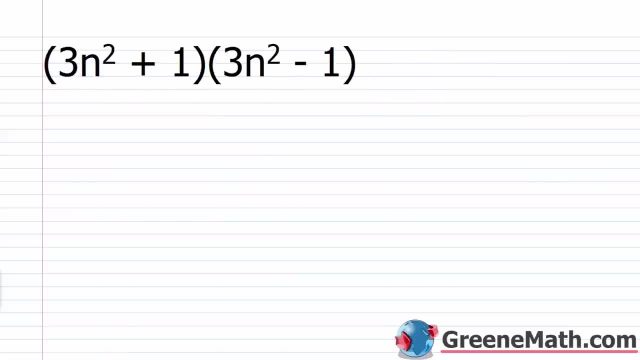 Alright, what about something like 3n squared plus 1 times 3n squared minus 1. So 3n squared, 3n squared. And then 1 and 1. So that works out. So we're going to take our first term, 3n squared, and we're going to square it. 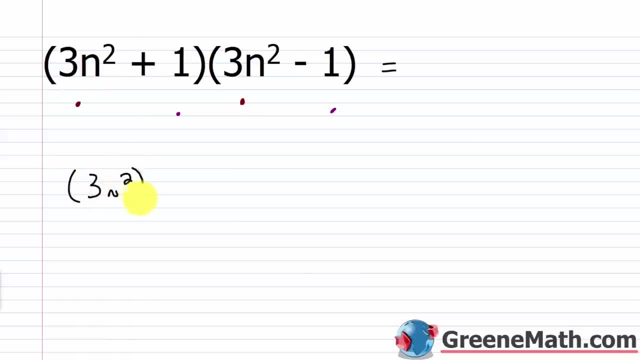 So think about this. 3n squared, and we're going to square it. So 3 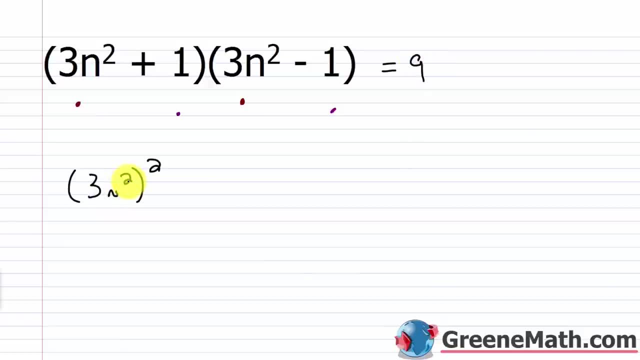 squared is easy. That's 9. What is n squared squared? 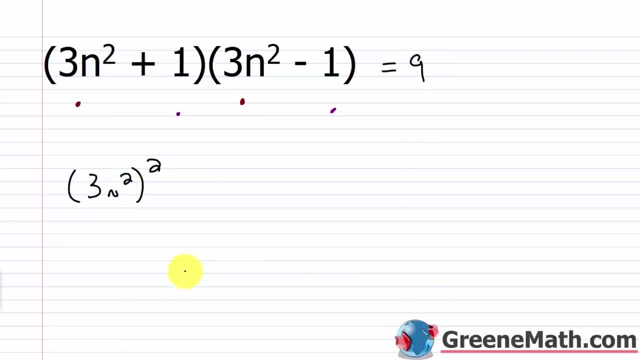 Alright, if I have n squared, that means I have n times n. And let's say I square that guy. Well that means that I'm going to have this twice. So I have n times n times n times n, or n to the fourth power. 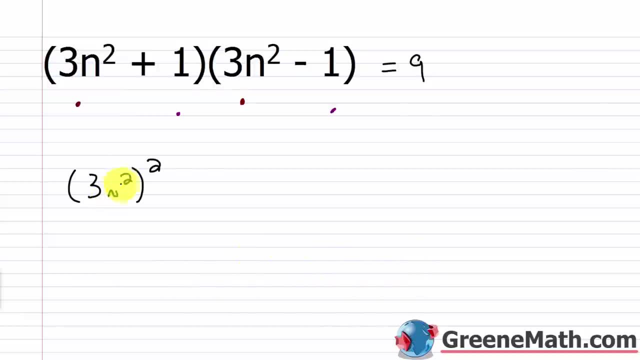 Again, this is found using the power to power rule. So I just take the base and leave it the same. And I multiply the exponents. So 2 times 2 would be 4. So this is n to the fourth power. Then I'm subtracting away. I have this term here, the second term. And that's going to be squared. 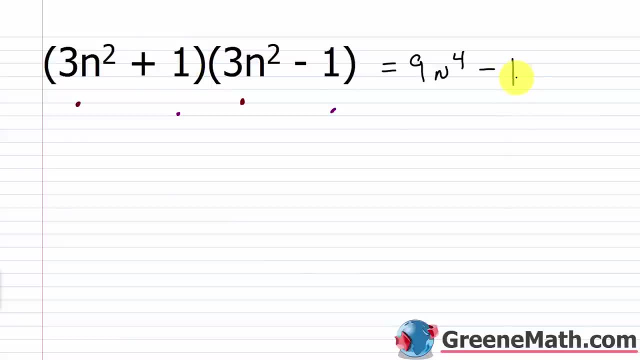 1 squared is 1. So we end up with 9n to the fourth power minus 1. 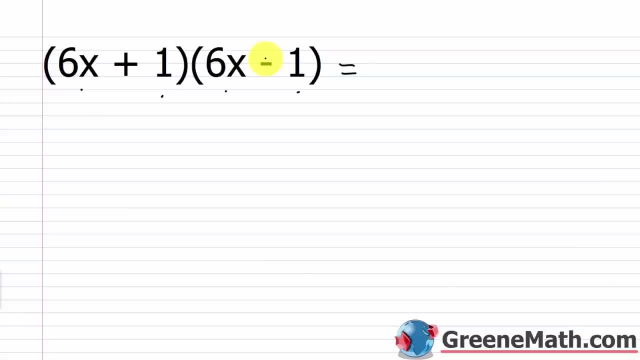 Just the plus and the minus is what's differing here. So then the first term is squared. Again, don't just write 6x squared. Don't just write 6x squared, 6 squared and move on. Very, very common mistake. 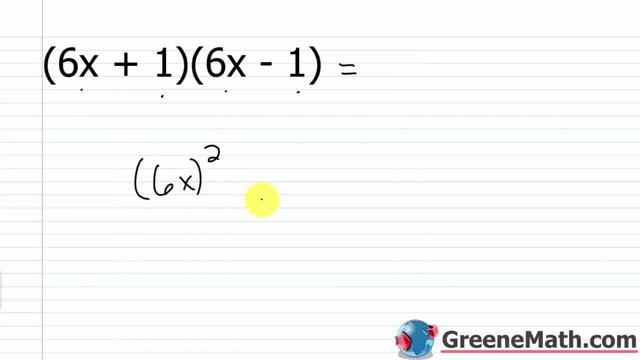 You've got to square the whole thing. The 6 and the x are both squared. 6 squared is 36.. X squared is x squared Then minus. I'm going to take that second term, which is 1, and I'm going to square that. 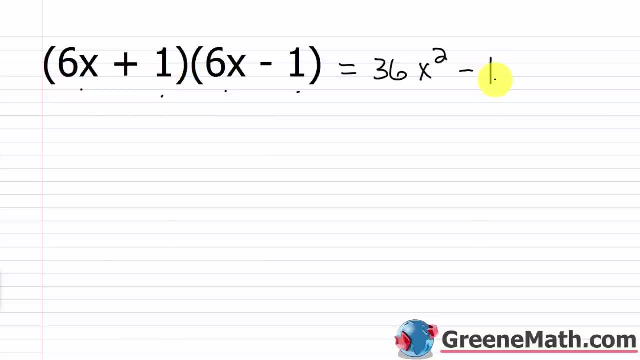 We all know 1 squared is just 1.. So this ends up being 36x squared minus 1.. And again, go through and use FOIL and verify that I got the right answer. Alright. what about something like 3n squared plus 1?? 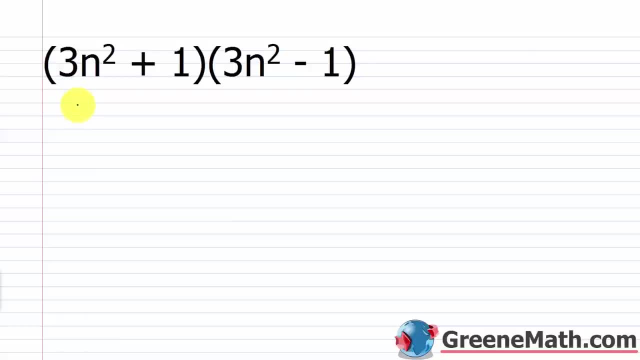 3n squared minus 1.. So 3n squared, 3n squared and then 1 and 1.. So that works out. So we're going to take our first term: 3n squared and we're going to square it. 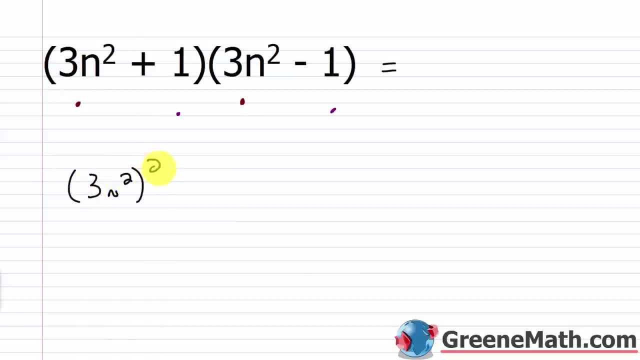 So think about this: 3n squared and we're going to square it. So 3 squared is easy, That's 9.. What is n squared squared Right? If I have n squared, that means I have n times 9.. 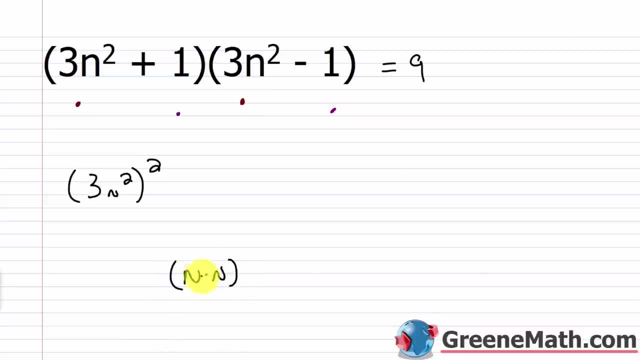 That's 2n squared, That's 3n squared, That's 2n squared times n. And let's say I square that guy. Well, that means that I'm going to have this twice. So I have n times, n times, n times n or n to the fourth power. 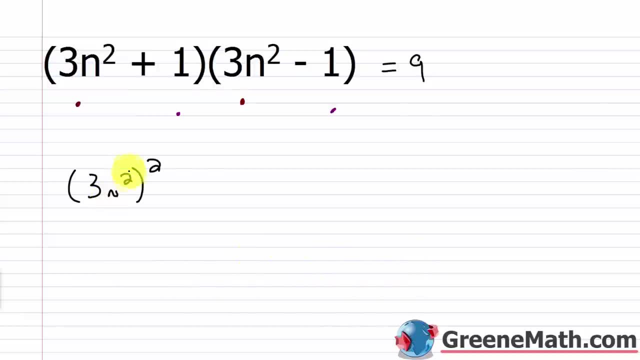 Again, this is found using the power-to-power rule, So I just take the base and leave it the same and I multiply the exponents. So 2 times 2 would be 4.. So this is n to the fourth power. 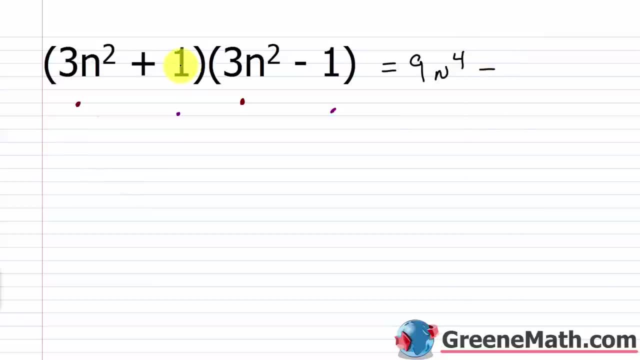 Then I'm subtracting away. I have this term here, the second term, And that's going to be squared 1. squared is 1.. with 9n to the fourth, power minus one. All right, what about something like x plus 1 1⁄2y? 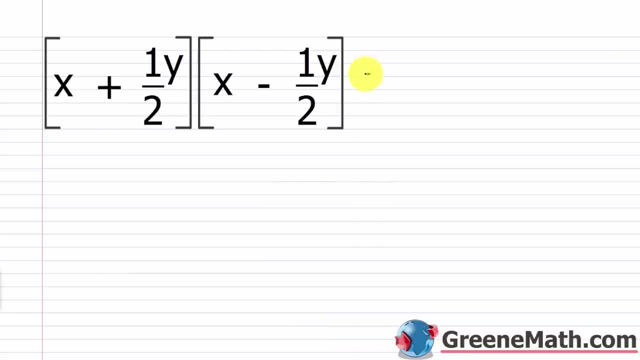 times x minus 1 1⁄2y. Well, again I'm looking at what's in the first position here I have x and I have x. What's in the second position? I have 1 1⁄2y and 1 1⁄2y. 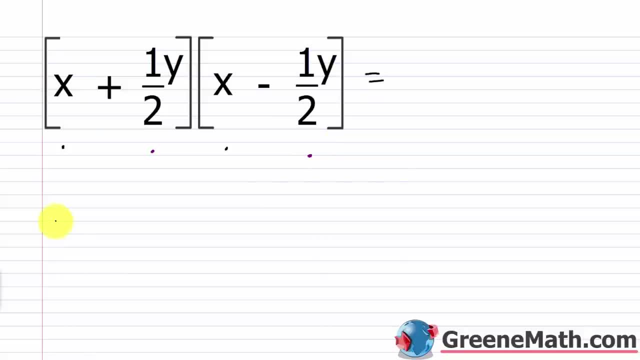 So we're good to go there. So I'm gonna take what's in the first position, which is x, and I'm gonna square it, And then I'm subtracting away what's in the second position and I'm gonna square that. 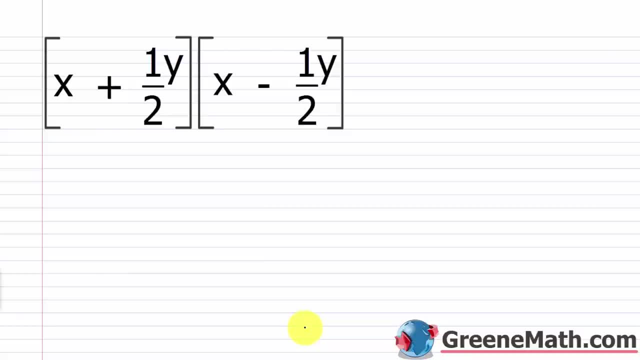 Alright, what about something like x plus 1 half squared? 1 half y times x minus 1 half y. 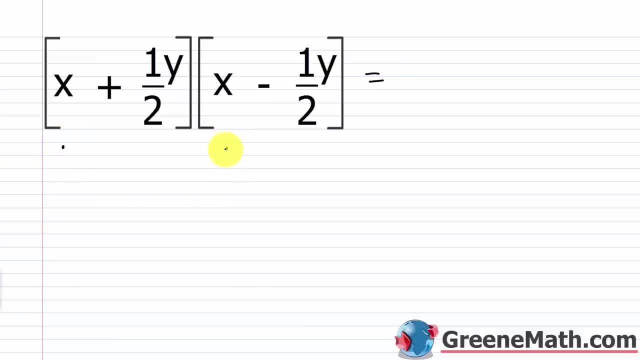 Well again, I'm looking at what's in the first position here. I have x and I have x. What's in the second position? I have 1 half y and 1 half y. 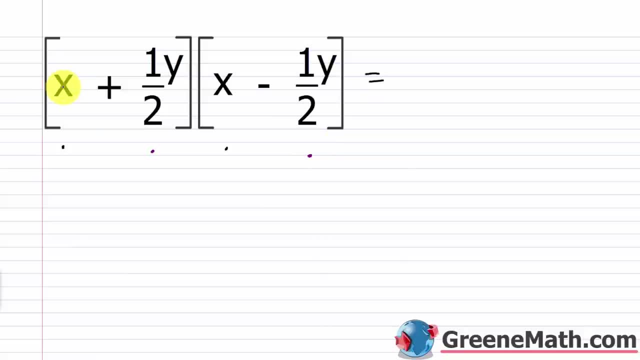 So we're good to go there. So I'm going to take what's in the first position, which is x, and I'm going to square it. And then I'm subtracting away what's in the second position, and I'm going to square that. So if I square 1 half y, if I square this whole thing, 1 half squared, 1 squared is 1. 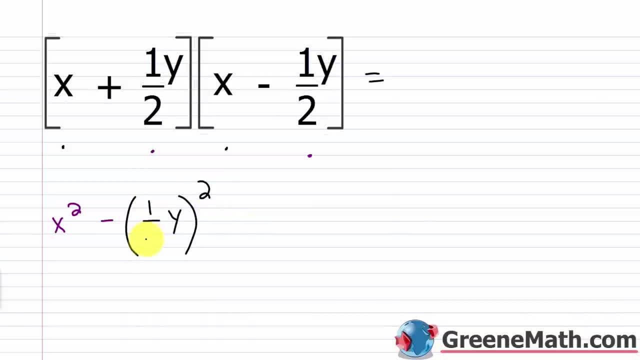 2 squared is 4. So this would be a 4 here. 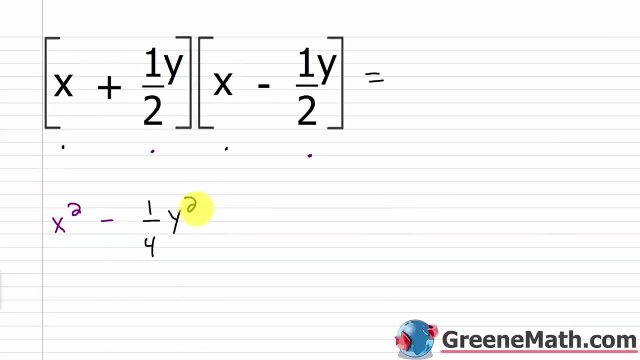 And we know that y squared is just y squared. So we end up with x squared minus 1 fourth y squared. Alright, what about 9m squared 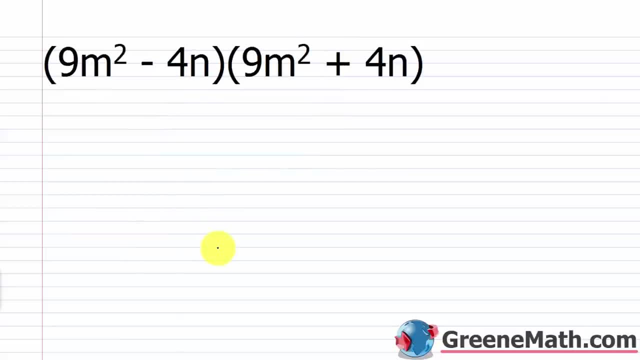 minus 4n times 9m squared plus 4n? 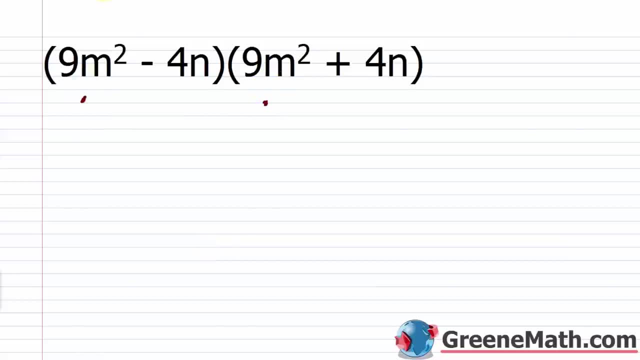 So again, 9m squared, 9m squared, and we're looking at 4n and 4n. So we're good to go there. 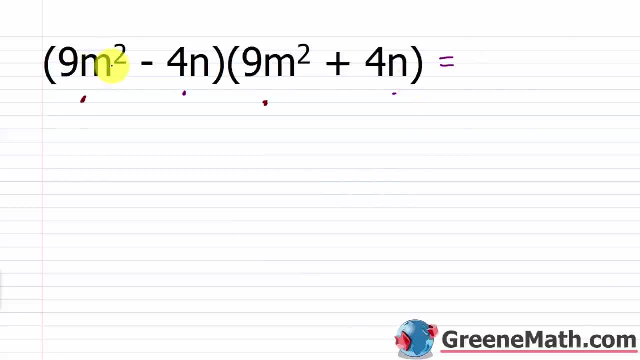 So we'll just start out. We have this first term, and that's going to be squared. 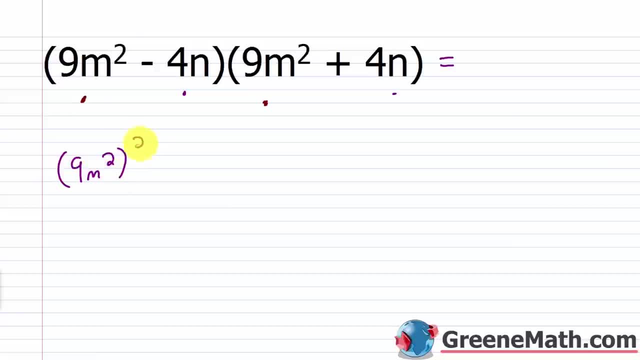 So 9m squared is going to be squared. 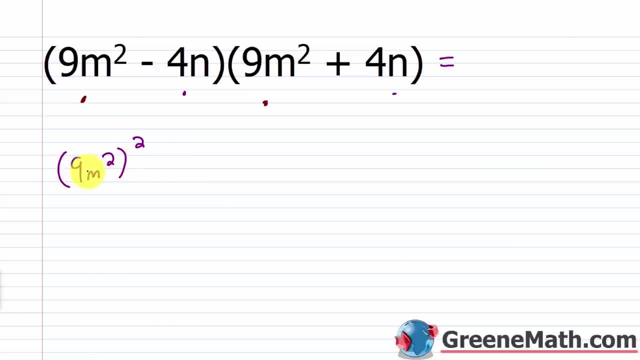 So what's that going to give me? Well, 9 squared is 81. 9 times 9 is 81. 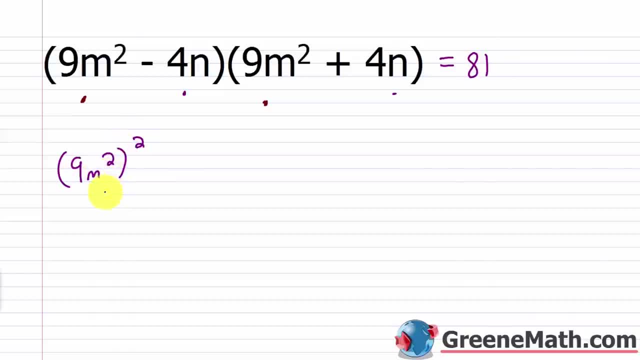 m squared raised to the power of 2. Again, use the power to power rule. Base m is going to stay the same. 2 times 2 is 4. Now I'm going to put a minus there. 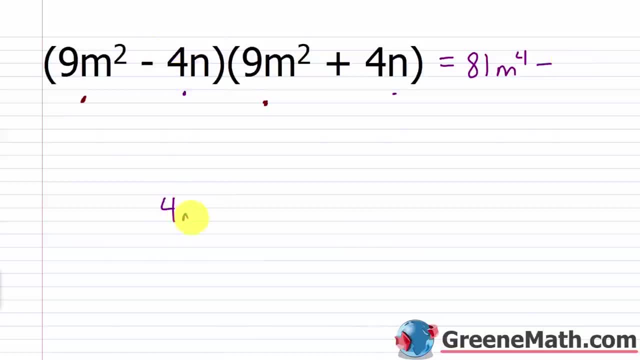 My second term is going to be squared. So I'm going to have 4n and that's going to be squared. So the 4 and the n are both squared. Again, very important you don't make that mistake. 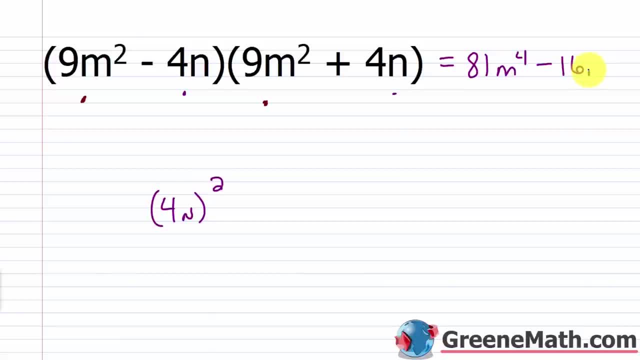 4 squared is 16. And then n squared is just n squared. So I'm going to end up with 81m to the fourth power minus 16n squared. 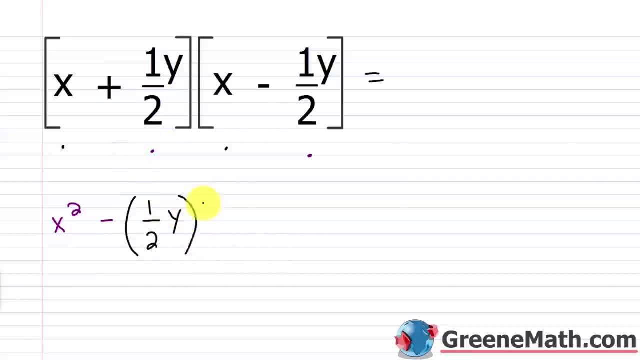 So if I square 1 1⁄2y, if I square this whole thing, 1 1⁄2 squared, 1 squared is one. two squared is four. So this would be a four here, And we know that y squared is just y squared. 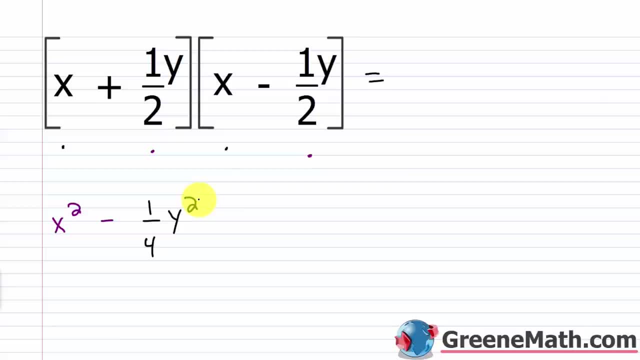 So we end up with x squared minus 1⁄4y squared. All right, what about 9m squared minus 4n times? 9m squared plus 4n, So again, 9m squared, 9m squared. 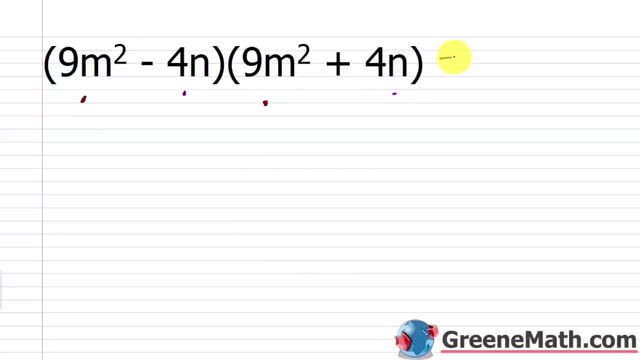 and we'll look at that. We're looking at 4n and 4n, So we're good to go there. So we'll just start out. We have this first term and that's gonna be squared. So 9m squared is going to be squared. 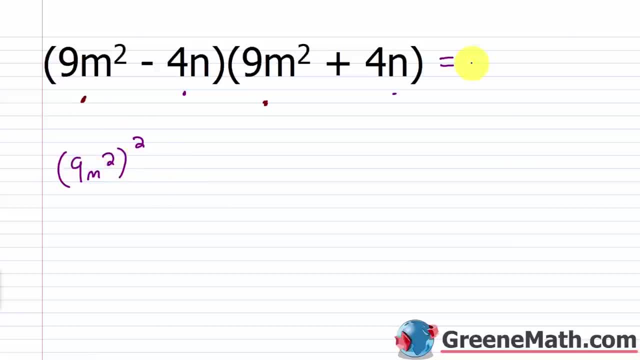 So what's that gonna give me? Well, 9 squared is 81, right Nine times nine is 81.. M squared raised to the power of two. Again, use the power to power. rule Base m is gonna stay the same. 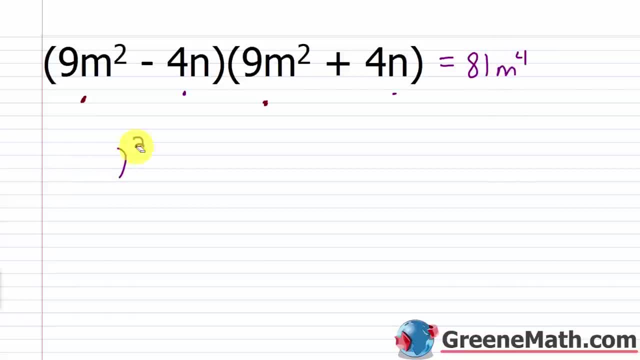 Multiply exponents Two times two is four. Now I'm gonna put a minus there. My second term is gonna be squared, So I'm gonna have 4n and that's gonna be squared. So the four and the n are both squared. 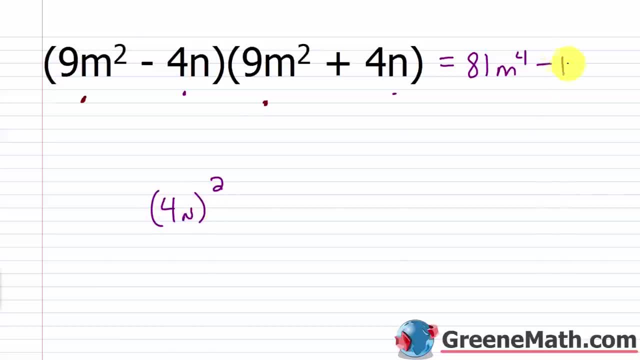 Again very important, you don't make that mistake: Four squared is 16, and then n squared is just n squared. So I'm gonna end up with 81m to the fourth power, minus 16n squared. All right. so, lastly, let's look at a binomial that is cubed. 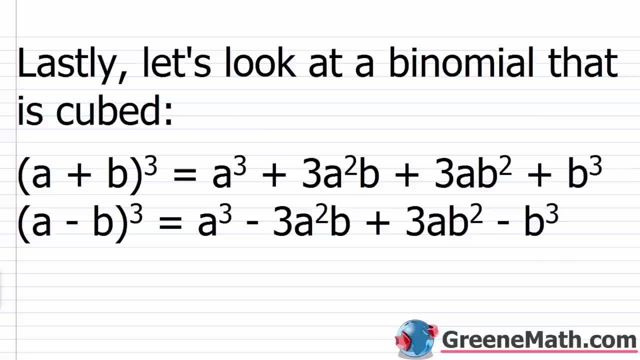 And this formula is a lot more difficult to memorize. The formulas I gave you up to this point- they're all the same. I gave you up to this point- are very easy. You can memorize them after about a day's worth of practice. 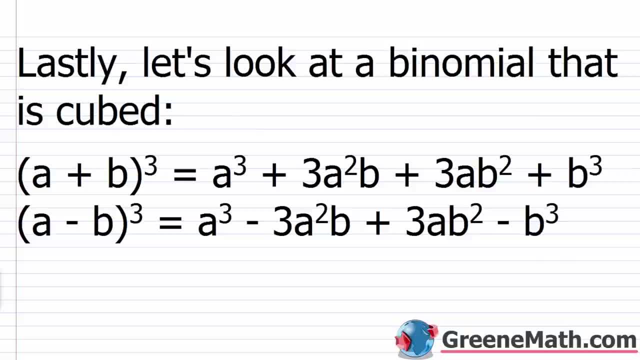 This one you kind of have to work on, but I'm gonna tell you that it's more rewarding and it saves you much more time to memorize these, Because when this comes up on an exam, if you've got this down packed, 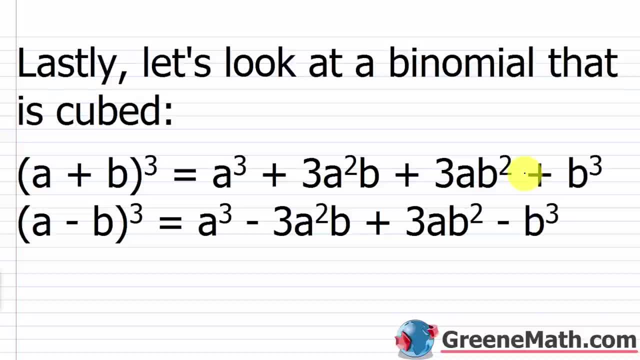 this is gonna save you a solid, let's say, minute and a half of you cranking stuff out at minimum right? So if you know these off the top of your head and you're confident in your ability to execute the formula, 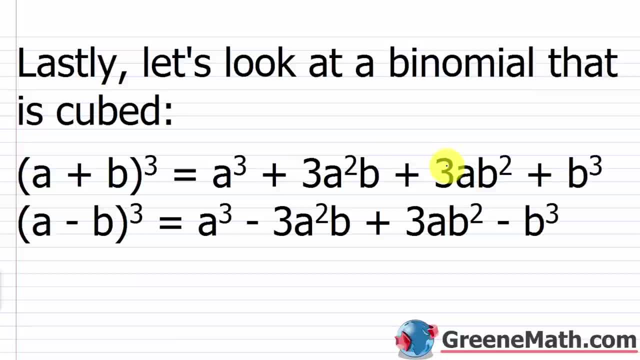 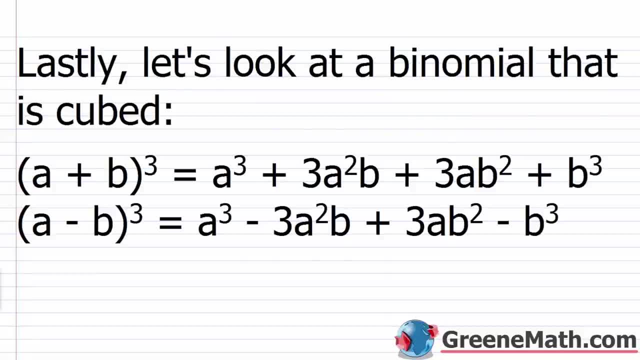 Alright, so lastly let's look at a binomial that is cubed. And this formula is a lot more difficult to memorize. 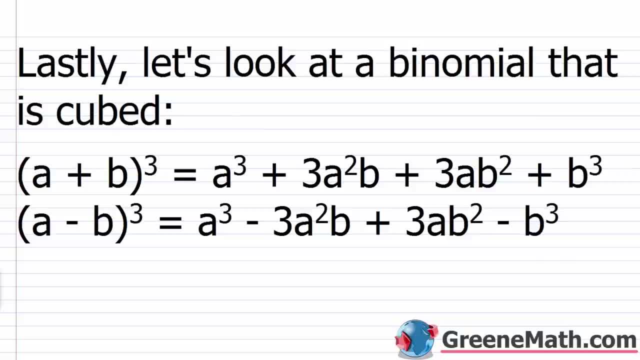 The formulas I gave you up to this point are very easy. You can memorize them after about a day's worth of practice. 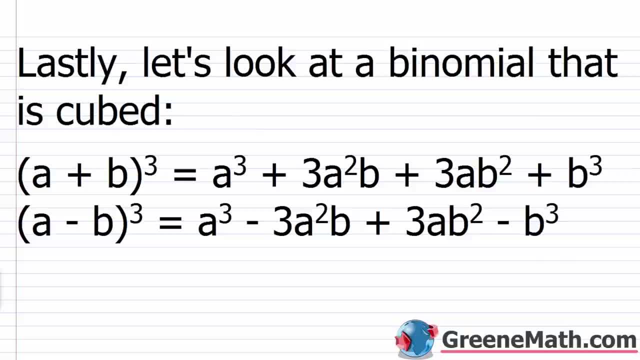 This one you kind of have to work on. But I'm going to tell you that it's more rewarding and it saves you much more time to memorize these. 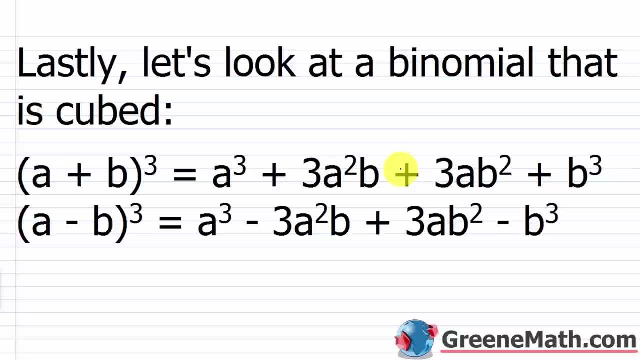 Because when this comes up on an exam if you've got this down packed this is going to save you a solid let's say minute and a half of you cranking stuff out at minimum. 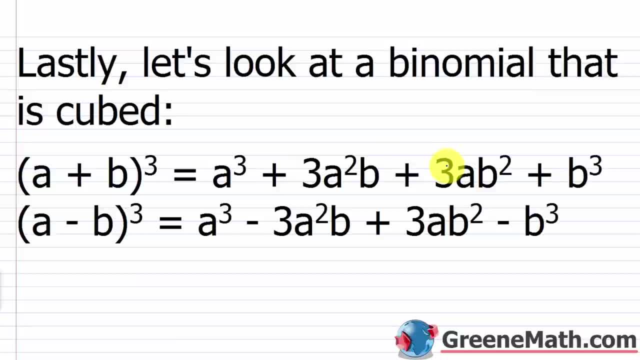 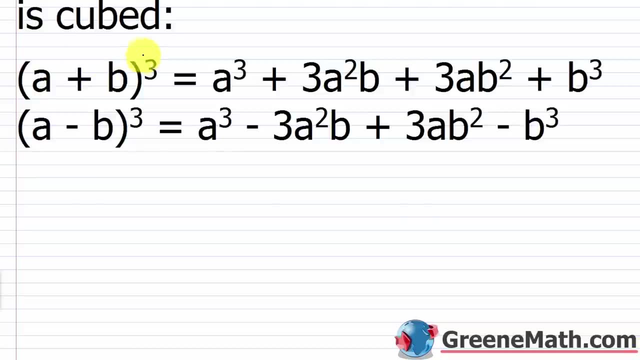 So if you know these off the top of your head and you're confident in your ability to execute the formula this is the biggest time saver that you're going to have for your kind of basic algebra one algebra two test that involves cubing a binomial. So I have that a plus b. That quantity is cubed. You get a cubed plus 3 times a squared b plus 3ab squared plus b cubed. 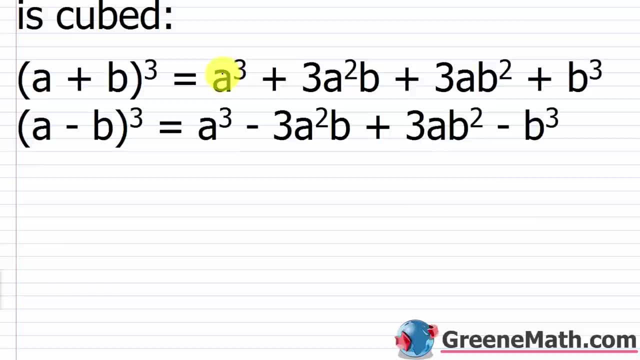 So essentially you have the first term cubed. Then you have 3 times the first term squared then times the second term. Then plus 3 times the first term times the second term squared plus the final term cubed. Now here's kind of the trick to remembering this. 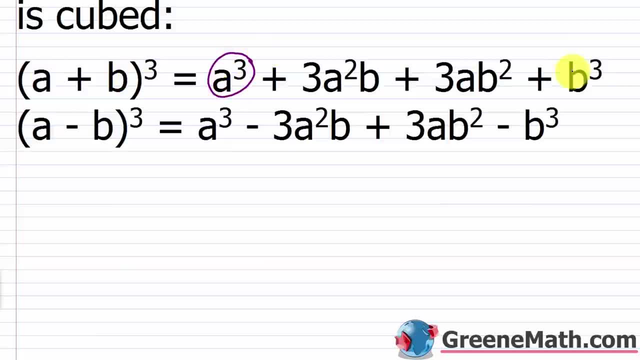 You know that you're going to have your first and your last term 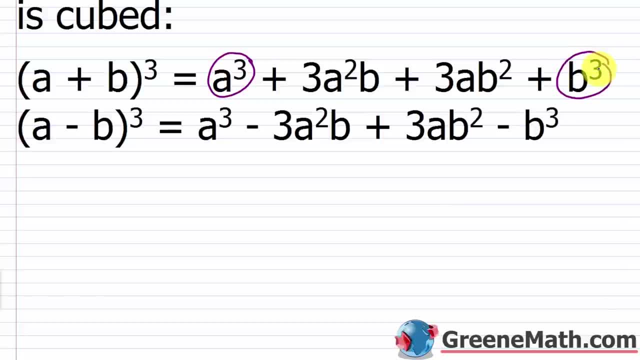 So what I do is if I can't remember I write those out first. 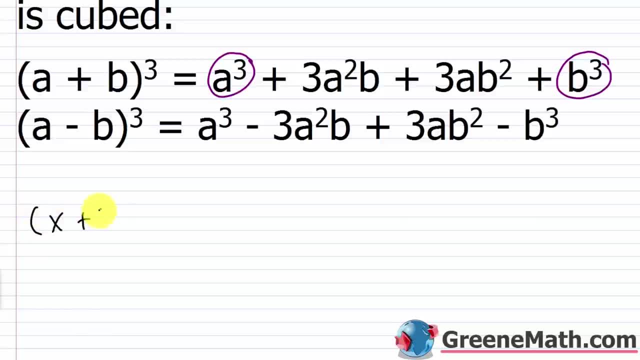 So let's say I had something like x plus 2 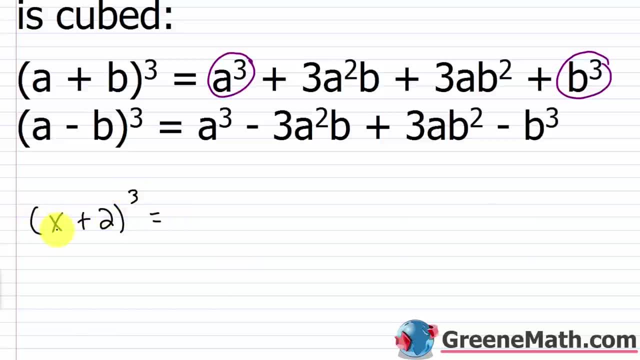 and that's cubed. So I know I'm going to have this first one cubed. So x cubed. 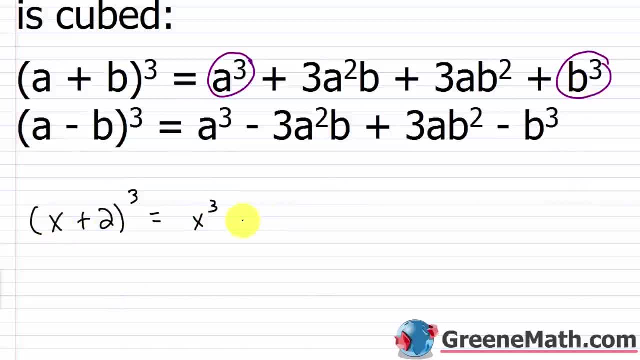 And I know I'm going to have the last one. The last one which is 2 cubed. So plus 2 cubed. cubed is going to be 8. Let me write that way down there. Now in between I can remember the number parts here because the cubed part is a 3. So I know I have 3 and space space and then plus 3 again space space. 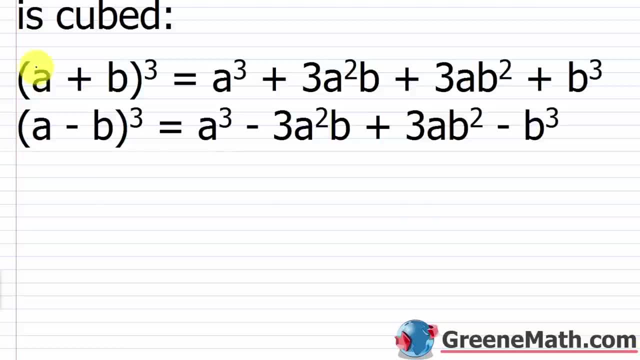 that involves cubing a binomial. So I have that a plus b. that quantity is cubed. You get a cubed plus 3 times a squared b plus 3ab squared plus b cubed. So essentially you have the first term cubed. 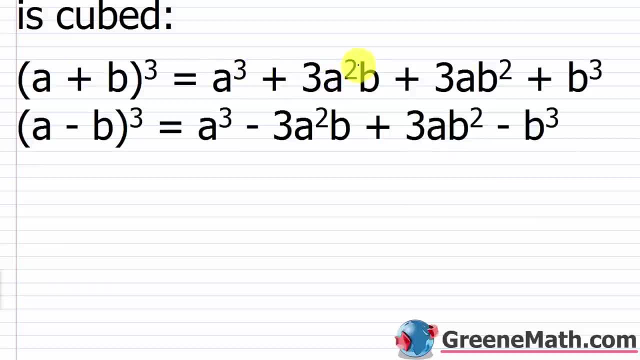 Then you have 3 times the first term squared, then times the second term, Then plus 3 times the first term, times the second term squared plus the final term cubed. Now here's kind of the trick to remembering this: You know that you're gonna have your first and your last term. that's going to be cubed. 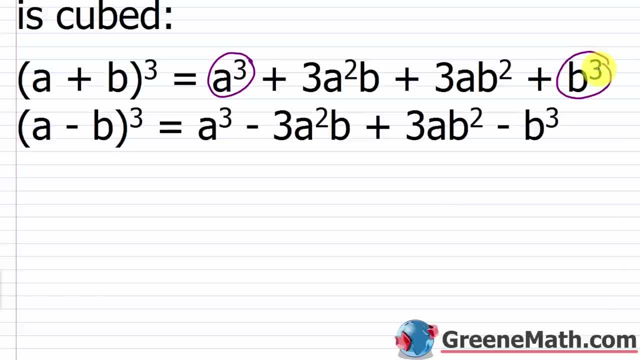 So what I do is, if I can't remember, I write those out first. So let's say I had something like I don't know, x plus 2 and that's cubed. So I know I'm gonna have this first one cubed. 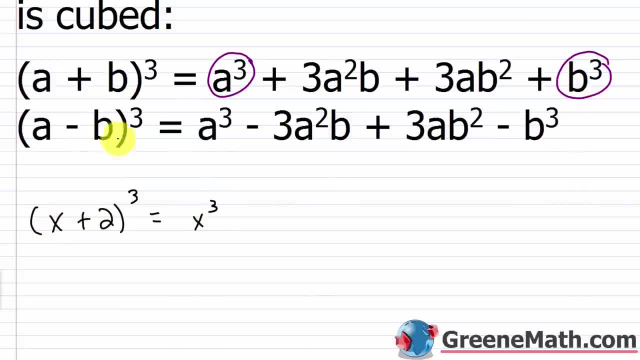 So x cubed, cubed, and I know I'm going to have the last one, the last one which is two cubed. so plus two cubed is going to be eight. let me write that way down there. now in between I can remember the number parts here because the cube part is a three. so I know I have three and space space. 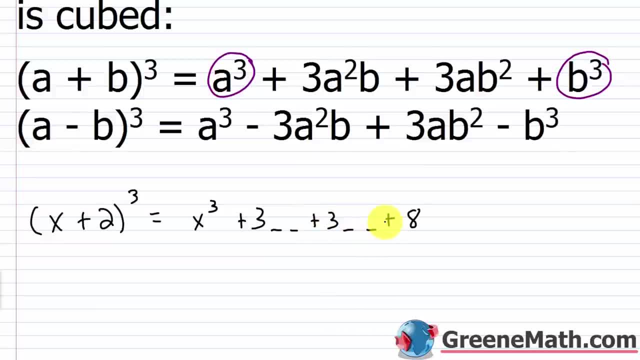 and then plus three, again space, space. now all you need to remember is that in each instance, one of them is going to be squared and one of them is not. so in other words, in the first instance, this first term is squared, so I get x squared and the second term is not. so times two and three: 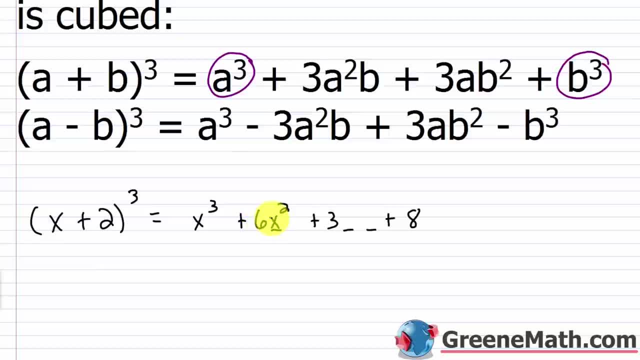 times two is six. so I can go ahead and erase this and put six for now. so six x squared. now, in the last one I put x squared the first term, so in this one I'm going to make the second term squared. so two squared is four. so this is going to be four and then the other one is going to be through the. 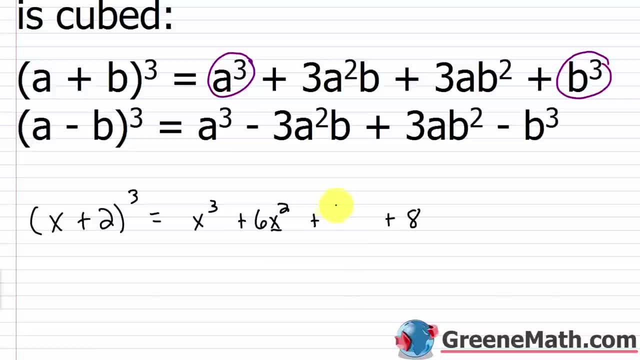 first power. so three times four is twelve. so this is going to be plus 12: x. so I get x cubed plus 6x squared, plus 12x plus 8, and that might not be the way you remember it, but this is always. if I get stuck for a minute, I remember that. okay, I know these first two, I know. 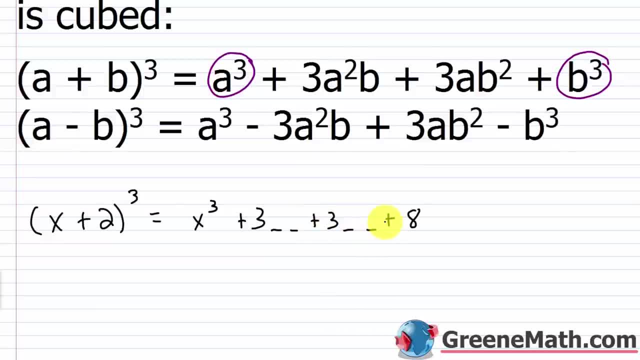 Now all you need to remember is that in each instance one of them is going to be squared and one of them is not. So in other words in the first instance this first term is squared so I get x squared and the second term is not. So times 2. And 3 times 2 is 6 so I can go ahead and erase this and put 6 for now. 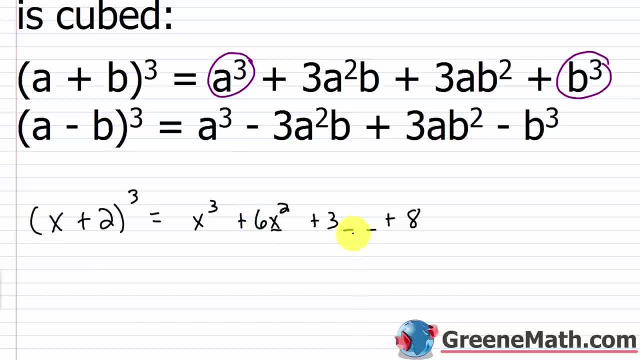 So 6x squared. Now in the last one I put x squared the first term. So in this one I'm going to make the second term squared. So 2 squared is 4. So this is going to be 4 and then the other one is going to be through the first power. So 3 times 4 is 12 so this is going to be plus 12x. So I get x cubed plus 6x squared plus 12x plus 8. And that might not be the way you remember it but this is always if I get stuck for a minute I remember that okay I know these first two. 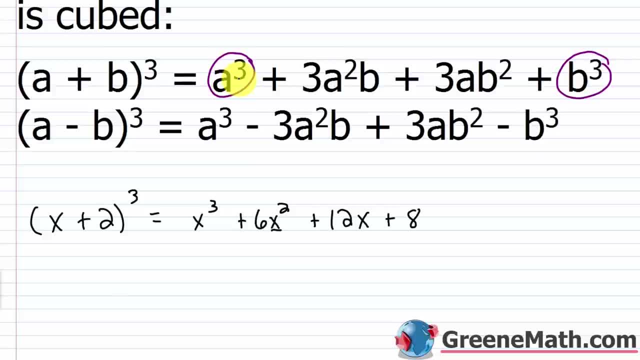 I know I'm going to have first term cubed second term cubed. And I know that I'm going to have two spaces each with a 3. And I know that each one of these is going to be used in those spaces. One's going to be squared in one instance. The other's going to be squared in the other instance. So once I remember that I just kind of go through a process of you know writing it out and then do that three or four times and then I'm good to go. 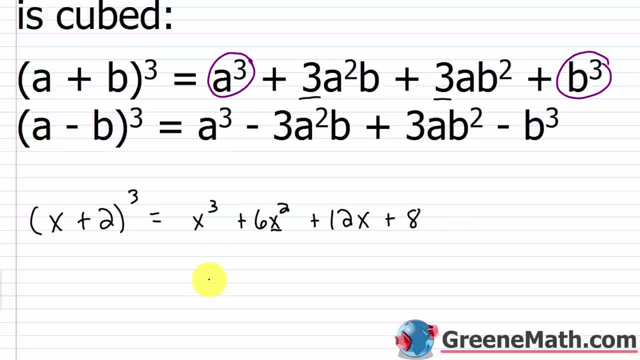 Now for the other one it's a little bit more difficult to remember. Because of the minus sign here you've got to remember that you have a minus sign here and then here. So it's right before the second term and right before the final term. So that's just something you have to remember. 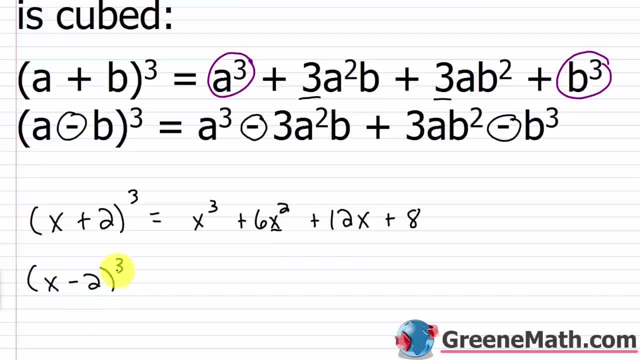 So for example if I had something like x minus 2 that cubed everything would be the same. 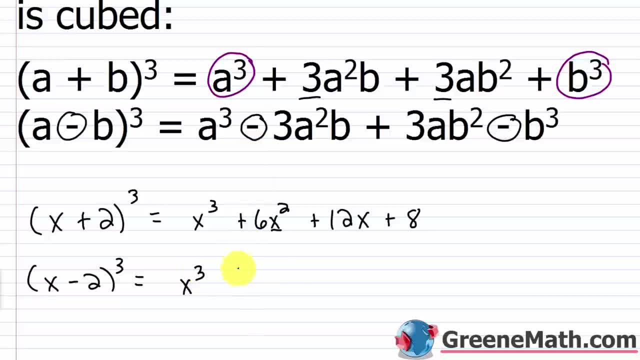 So I would have x cubed but then the signs would be different. So this would be minus 6x squared plus 12x and then minus 8. Alright so let's take a look at an example. 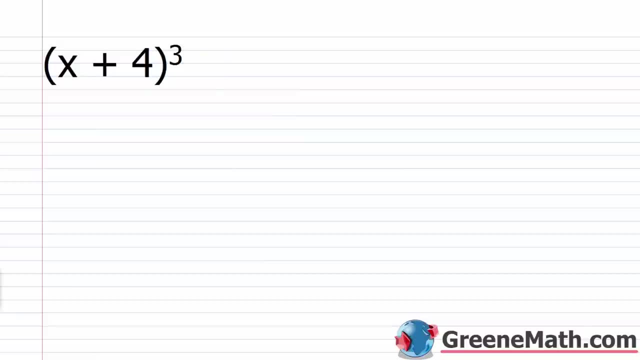 We have x plus 4 this quantity cubed. So again I know that I'm going to have this first one cubed and I know I'm going to have the last one cubed. 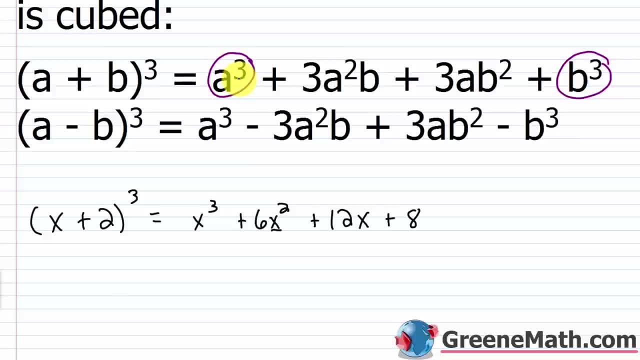 I'm going to have first term cubed, second term cubed, and I know that I'm going to have two spaces, each with a three, and I know that each one of these is going to be used in those spaces. one's going to be squared in one instance, the other is going to be squared in the other instance. so 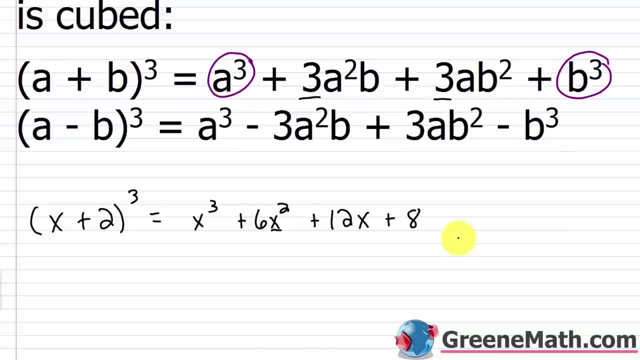 once. I remember that I just kind of go through a process of you know writing it out and then do that three or four times and then I'm good to go. now for the other one. it's a little bit more difficult to remember because of the minus sign here. you got to remember that you have a minus. 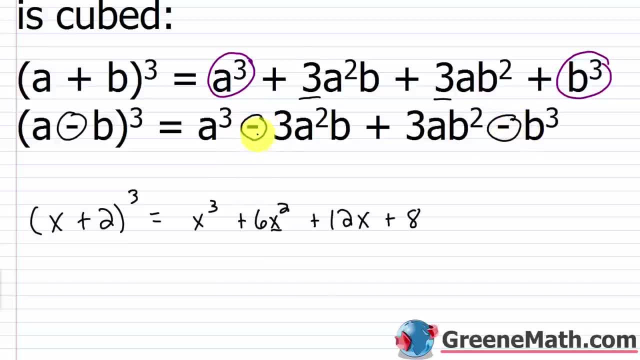 sign here and then here. so it's right before the second term and right before the final term. so that's just something you have to remember. so, for example, if I had something like x minus two that cubed, everything would be the same. so I would have x cubed. 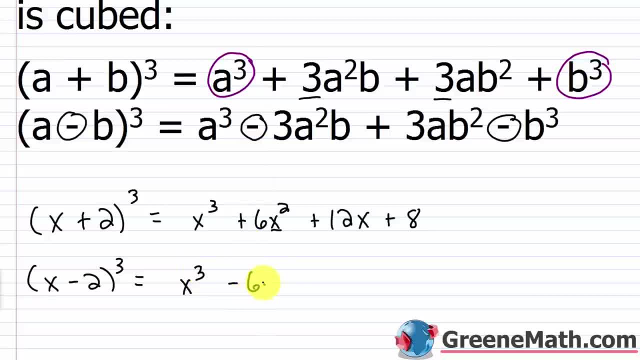 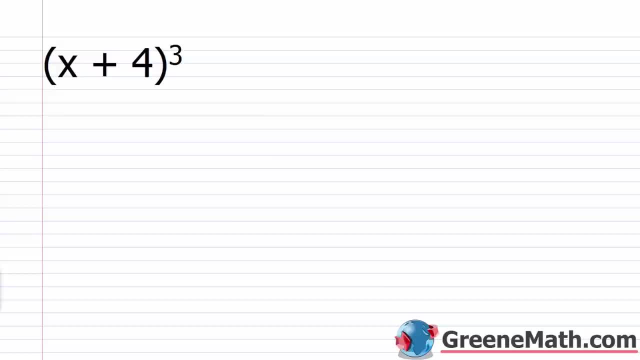 but then the signs would be different. so this would be minus six x squared, plus 12 x, and then minus eight. all right, so let's take a look at an example. we have x plus four, this quantity cubed. so again, I know that I'm going to have this first one cubed and I know I'm going to have the last. 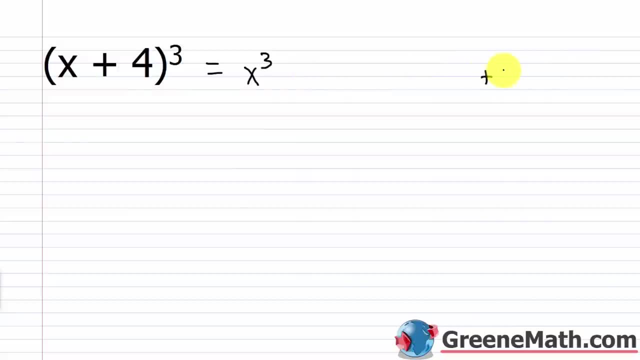 one cubed. so let's write that way over here. let's put plus four cubed. we'll go through and do the math in a little while. we know that four cubed is four times four, which is 16 times four again, which is 64.. 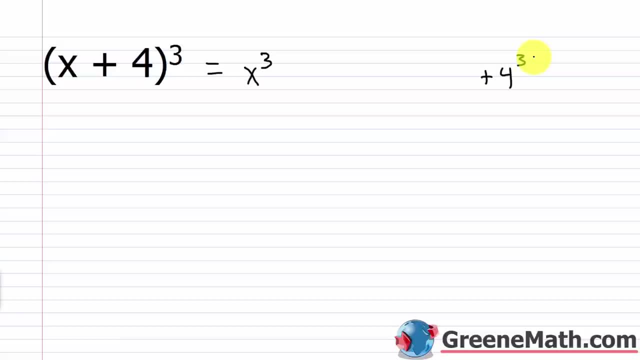 We'll just leave it as four cubed for now. now I know that I'm going to have plus something, plus something else. right, let me kind of scoot this down a little bit now. just think about this right here. this is going to be my number, so three and three. then just think about these two. one of them. 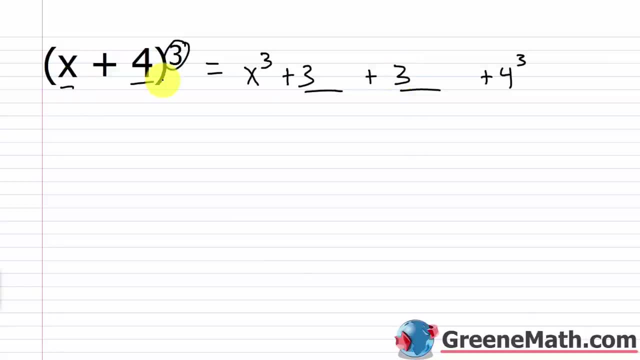 is going to be squared in one case and the other is going to be squared in the other case. so in other words, in the first case it doesn't matter the order that you do this in. so I could say: in the first case I'll just square the first one, so x squared and the second one won't be squared. so 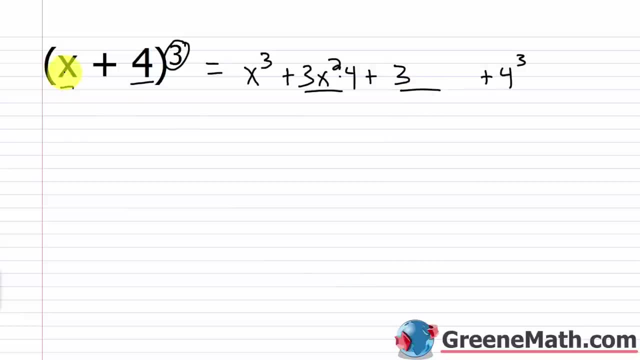 times four. then in the second case the four is going to be squared. so times four squared times x. now this one's not squared. so again, this is kind of how I remember it. it's, it's my thought process. you can use it or, you know, you can come up with something on your own, or maybe there's. 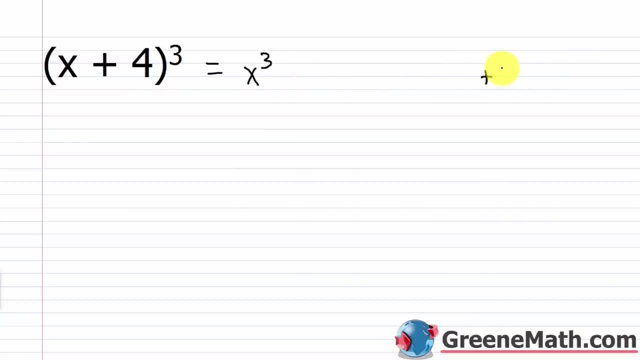 So let's write that way over here. Let's put plus 4 cubed. We'll go through and do the math in a little while. We know that 4 cubed is 4 times 4 which is 16 times 4 again which is 64. We'll just leave it as 4 cubed for now. 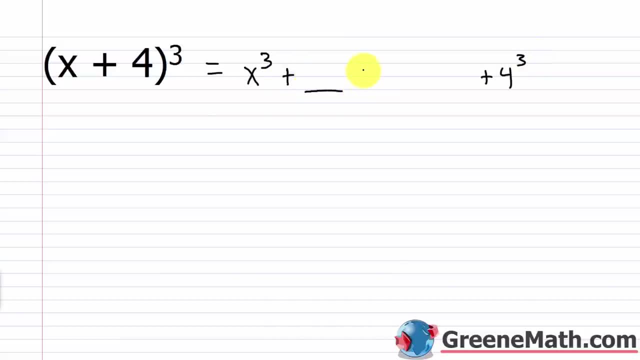 Now I know that I'm going to have plus something plus something else. Right? Let me kind of scoot this down a little bit. 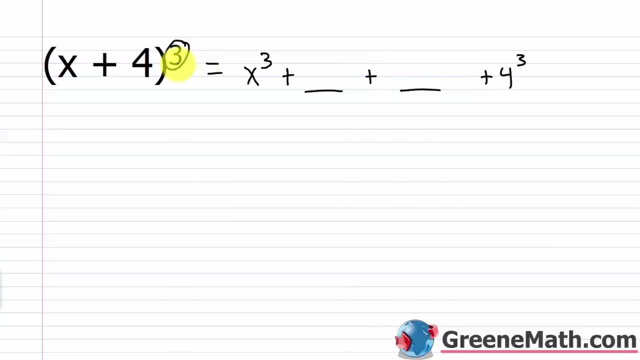 Now just think about this right here. This is going to be my number. So 3 and 3. Then just think about these two. One of them is going to be squared in one case and the other is going to be squared in the other case. So in other words in the first case it doesn't matter the order that you do this in. 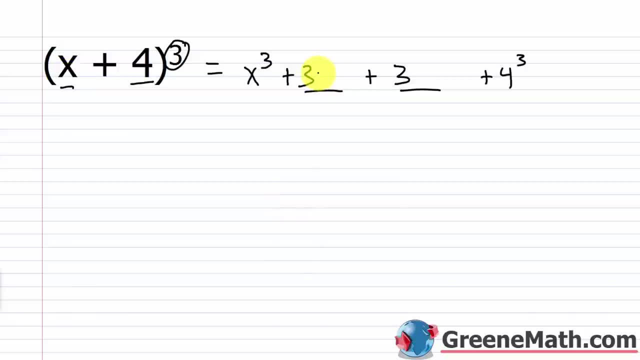 So I can say in the first case I'll just square the first one. So x squared and the second one won't be squared. So times 4. 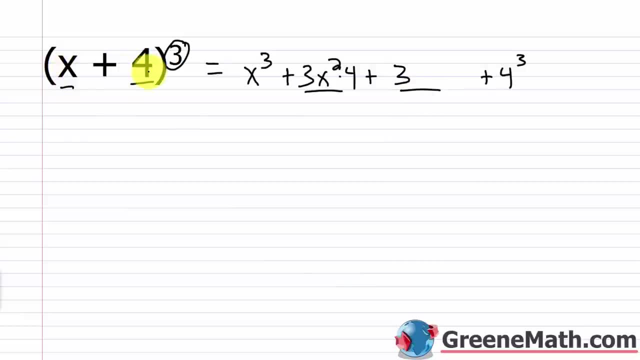 Then in the second case the 4 is going to be squared. 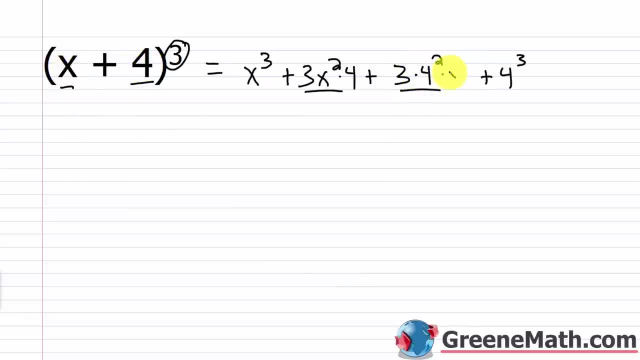 So times 4 squared times x. Now this one's not 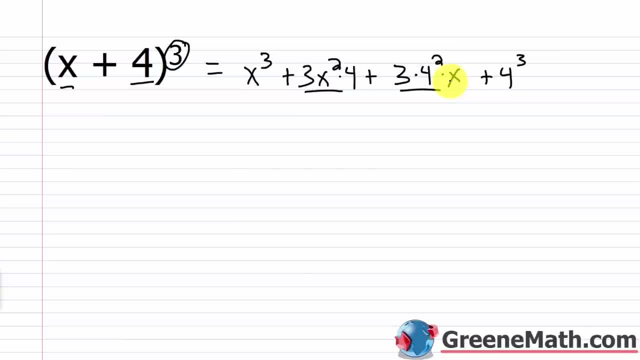 squared. So again this is kind of how I remember it. It's my thought process. You can use it or 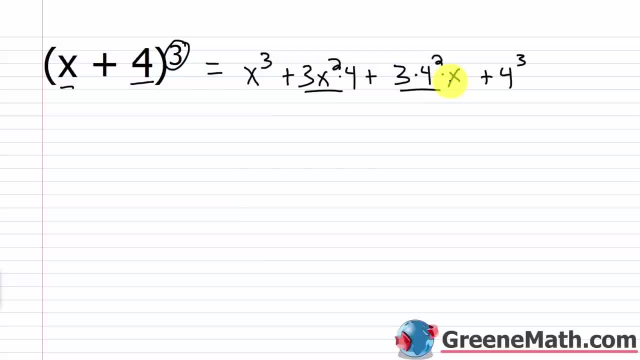 you can come up with something on your own or maybe there's another tutorial out there that makes more sense for you but this is how I remember it personally. So then I go through 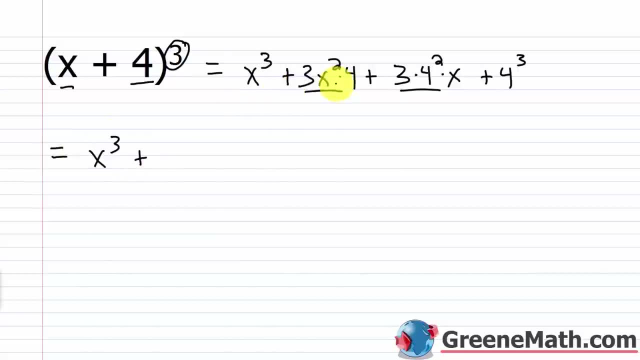 and just simplify. So then x cubed plus 3 times 4 is 12 so 12x squared plus 3 times we have 4 squared. 4 squared is 16. 3 times 16 is 48. So that's 48 x and then plus 4 cubed which is 64. 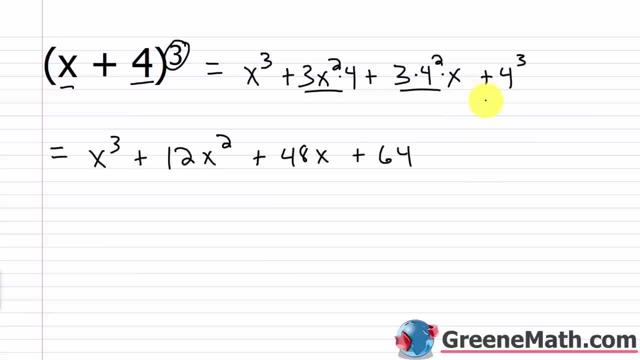 So that's your answer and you know if I didn't sit there and kind of write things out if I was on a test and kind of did that in my head I would probably have that answer in under 10 seconds. 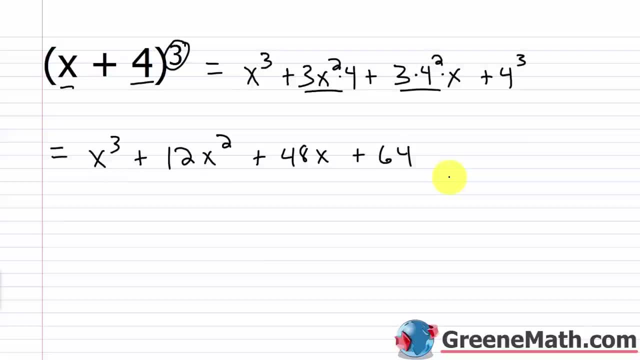 Right? Whereas if I went through and had to expand this right here this x plus 4 cubed let's just think about how long this takes. You have x plus 4 times x plus 4 times x plus 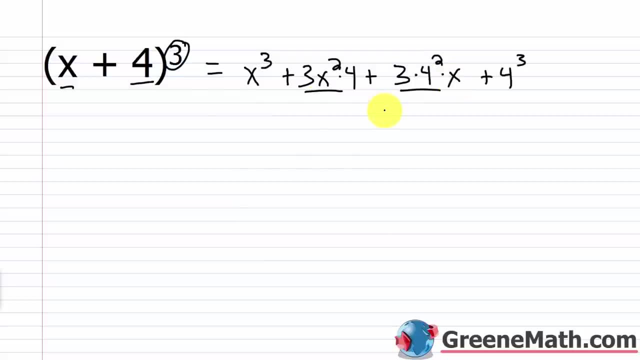 another tutorial out there that makes more sense for you, but this is how I remember it personally, so then I go through and just simplify. So then, x cubed plus 3 times 4 is 12, so 12x squared plus 3 times, we have 4 squared 4. 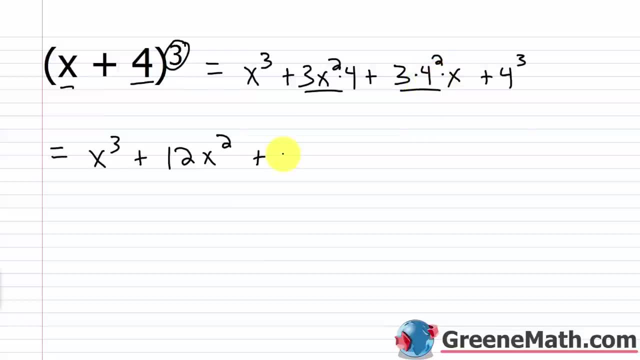 squared is 16, 3 times 16 is 48,, so that's 48x, and then plus 4 cubed, which is 64.. So that's your answer And you know, if I didn't sit there and kind of write things out, if I was on a test and 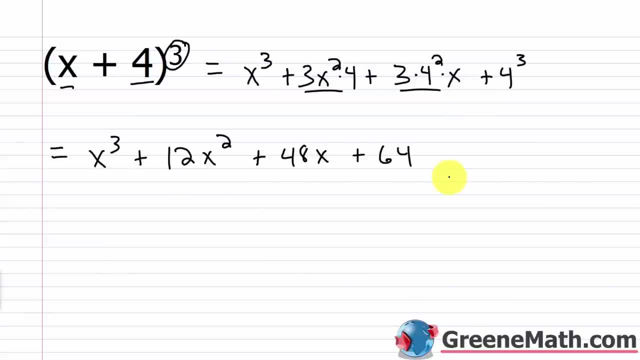 kind of did that in my head, I would probably have that answer in under 10 seconds, right? Whereas if I went through and had to expand this right here, this x plus 4 cubed- let's just think about how long this takes. 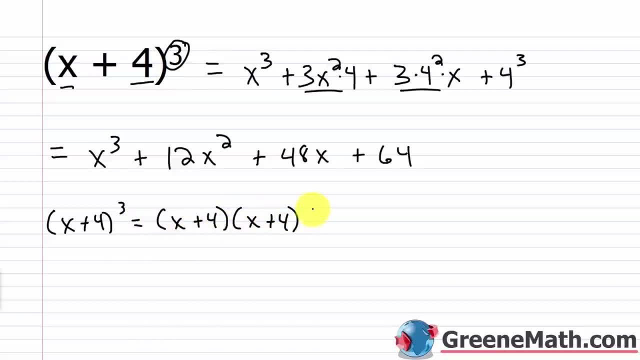 You have x plus 4 times x plus 4 times x plus 4.. Well, I could save myself a little bit of time, because remember this right here is the same thing as x plus 4, squared right. So I already know what that is. 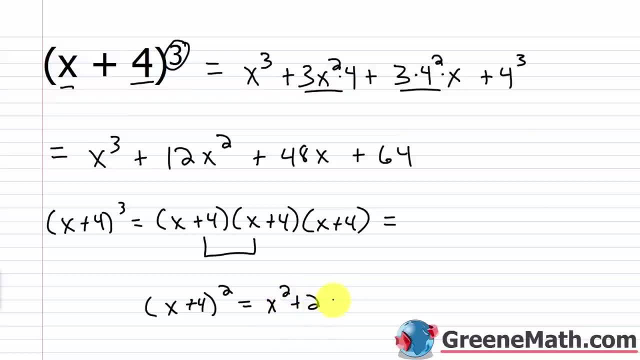 That's x squared Plus 2 times 4, which is 8, times x. so 8x plus 4 squared, which is 16.. So I could save myself a little bit of time with that, you know, just using that formula. 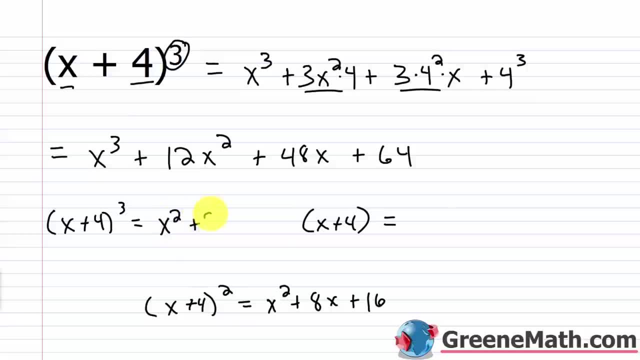 So this is x squared plus 8x plus 16, but I've still got to go through and multiply this guy by this guy. So I've got to do x times x squared. So x times x squared is x cubed. I've got to do x times 8x. 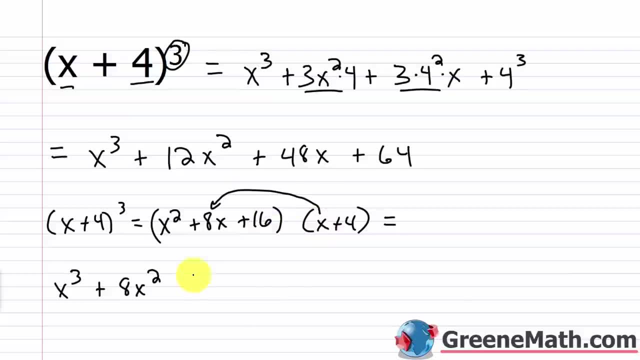 That's going to be plus 8x squared. I've got to do x times 16.. That's plus 16x, And then I've got to do 4 times this. So 4 times x squared is plus 4x squared. 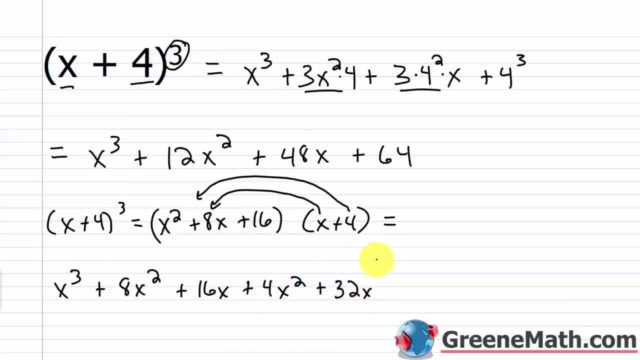 4 times 8x is plus 32x. 4 times 16 is plus 64.. So now I would combine like terms. So I have x cubed plus 8x squared. plus 4x squared is going to give me 12x squared, then plus 16x, plus 32x is 48x and then plus 64.. 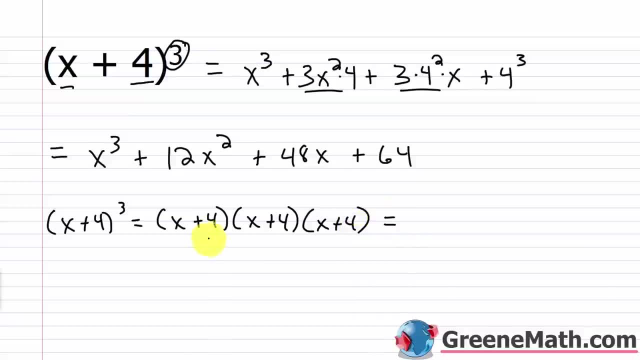 4. Well I could save myself a little bit of time because remember this right here is the same thing as x plus 4 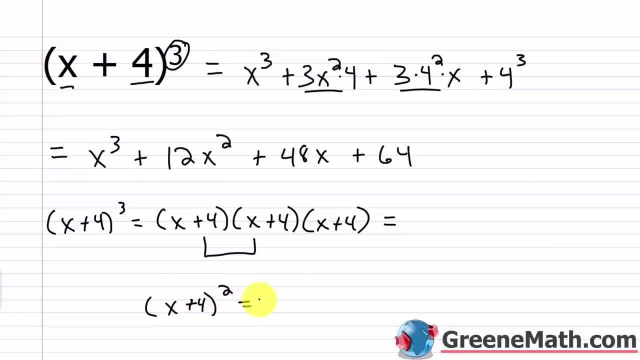 squared. Right? So I already know what that is. 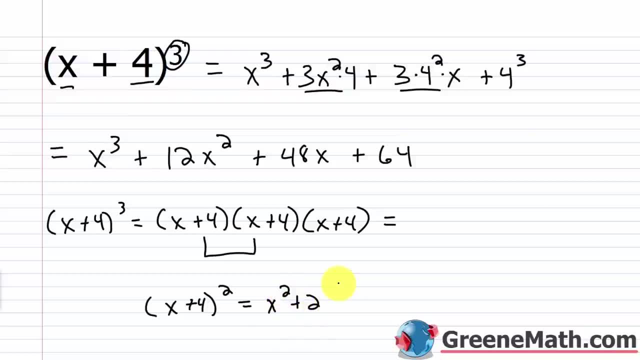 That's x squared plus 2 times 4 which is 8 times x so 8x plus 4 squared which is 16. So I could save myself a little bit 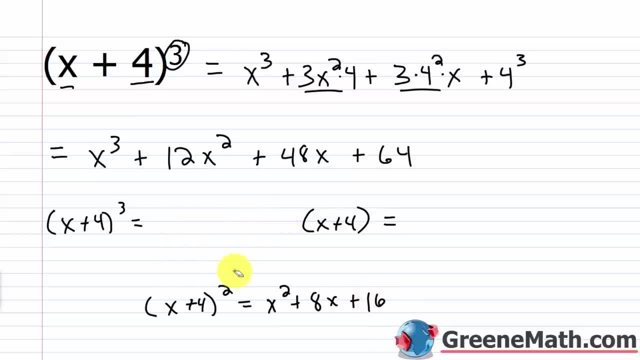 of time with that. You know just using that formula. So this is 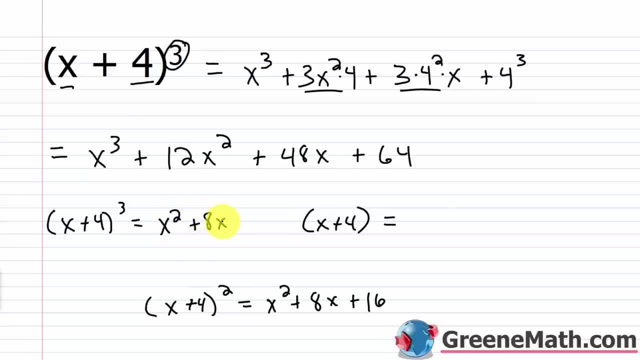 x squared plus 8x plus 16. But I've still 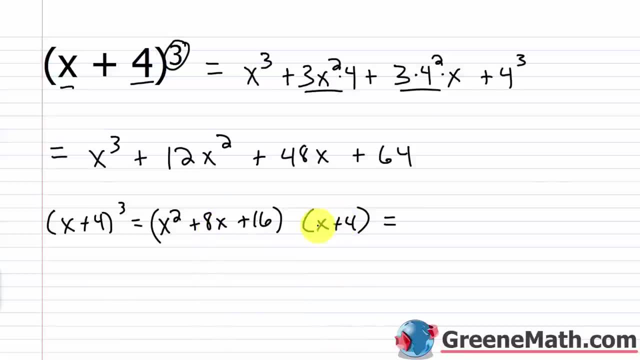 got to go through and multiply this guy by this guy. So I've got to do x times x 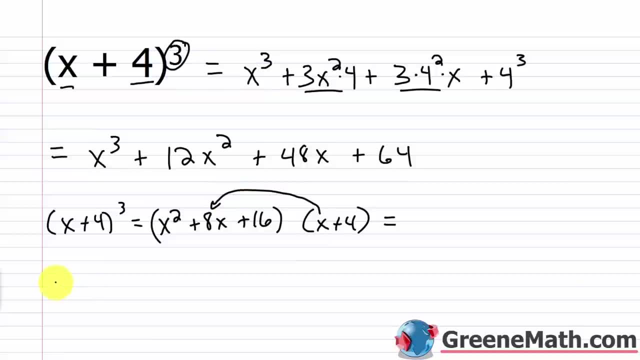 squared. So x times x squared is x cubed. 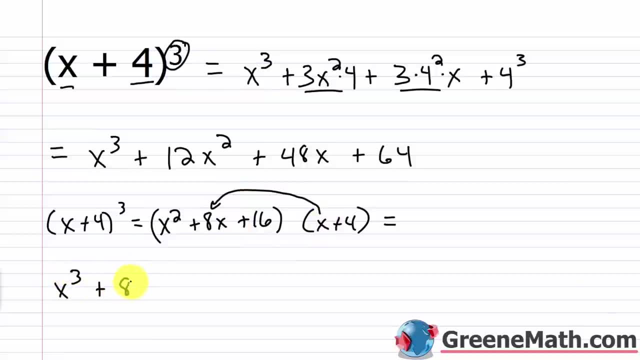 I've got to do x times 8x. That's going to be plus 8x squared. 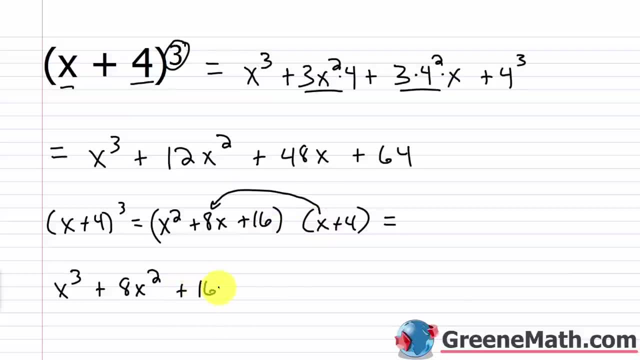 I've got to do x times 16 that's plus 16x. And then I've got to do 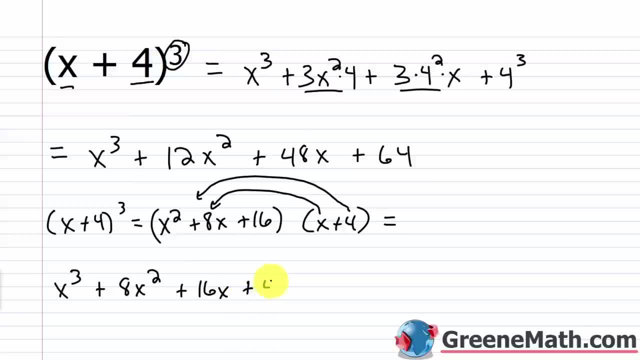 4 times this. So 4 times x squared is plus 4x squared. 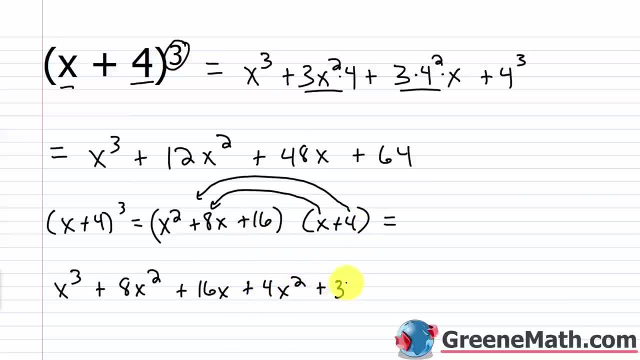 4 times 8x is plus 32x. 4 times 16 is plus 64. 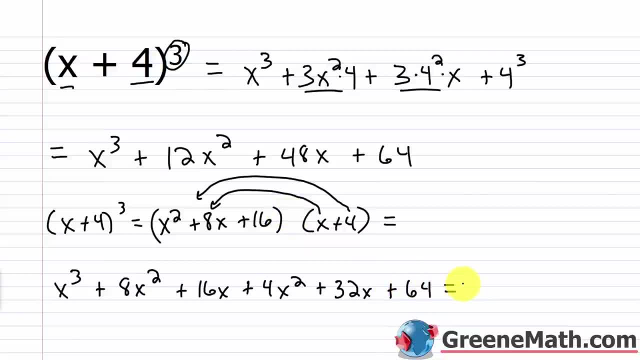 So now I would combine like terms. So I have x cubed plus 8x squared plus 4x squared is going to give me 12x squared. 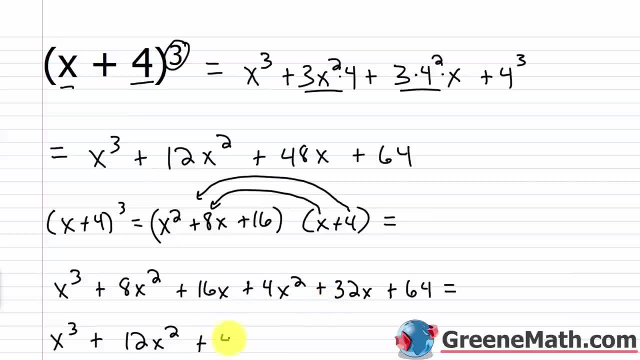 Then plus 16x plus 32x is 48x. 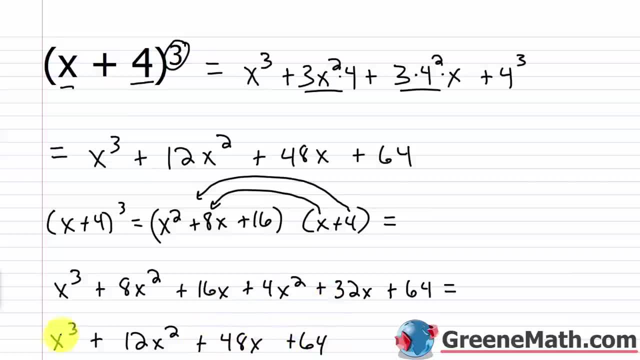 And then plus 64. So I got the same answer 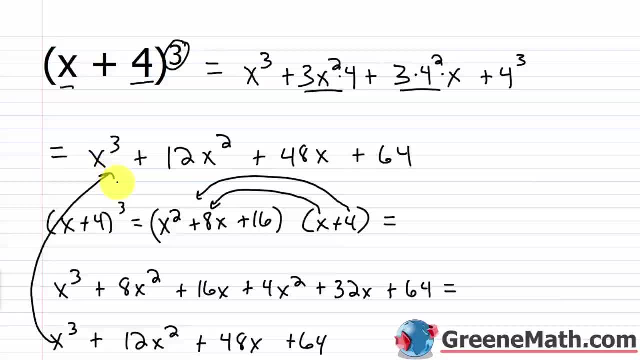 here but it took me a lot longer. And remember I still used a shortcut. I still went through and said okay I know that part of this x plus 4 times x plus 4 I already know the formula for that. 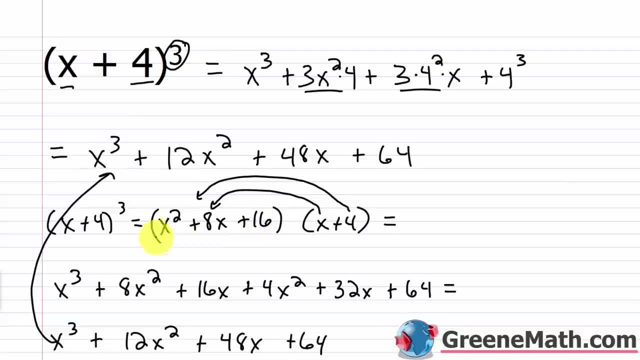 So if I had went through and did FOIL for that first to get this first kind of answer that would have taken even longer. So you can see already 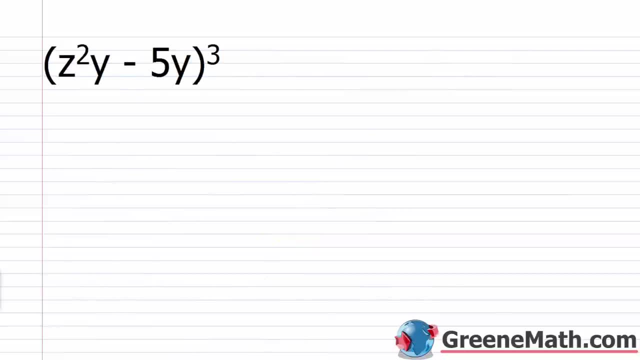 what a tremendous time saver this is going to be for you. Alright so now let's take a look at z squared y minus 5y and this guy is cubed. So again just trying to get a process for you to remember this. 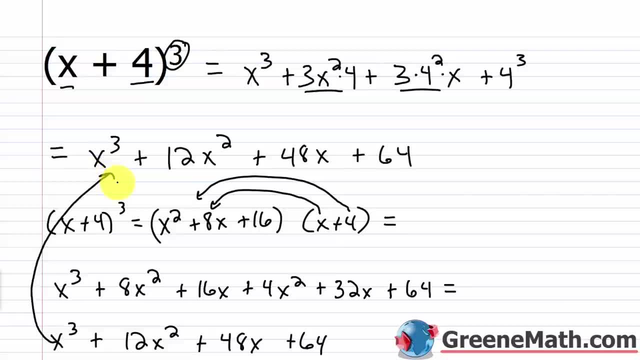 So I got the same answer here, but it took me a lot longer And remember I still used a shortcut. I still went through and said, okay, I know that part of this, x plus 4 times x plus 4,. 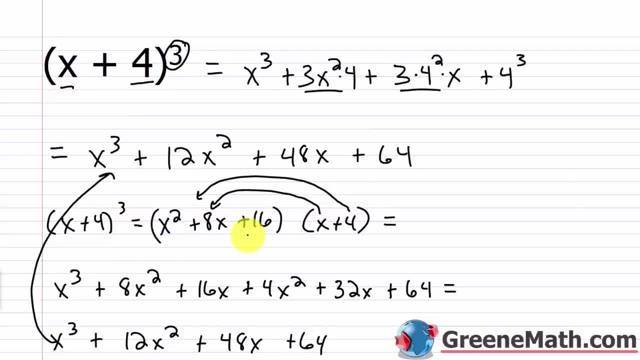 I already know the formula for that. So if I had went through and did FOIL for that first to get this first kind of answer, that would have taken even longer. So you can see already what a tremendous amount of time I have, what a tremendous time saver this is gonna be for you. 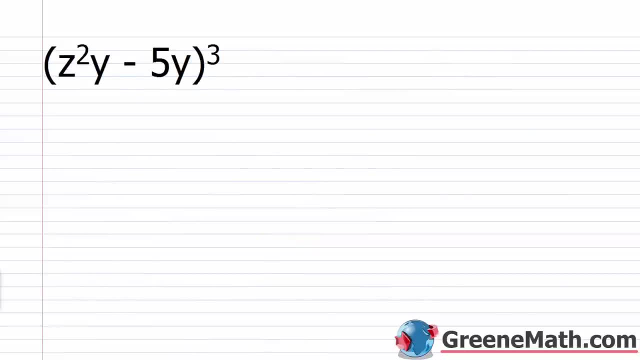 All right. so now let's take a look at z squared y minus five y, and this guy is cubed. So again, just trying to get a process for you to remember this: You'll always remember that the first guy, the first guy, is going to be cubed. 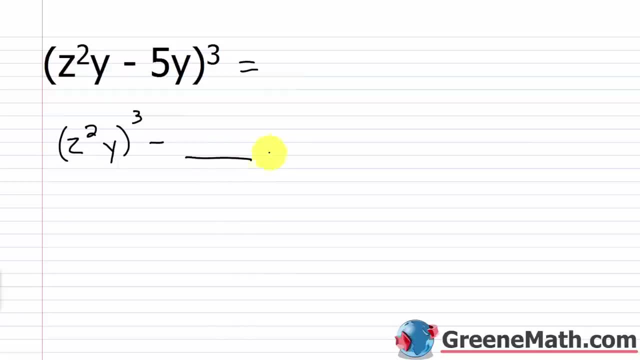 Now the second term. you have a space, then plus. you have a space, then minus. Remember your signs Before the second term and before the final term. So the final term is this guy right here, the five y cubed. 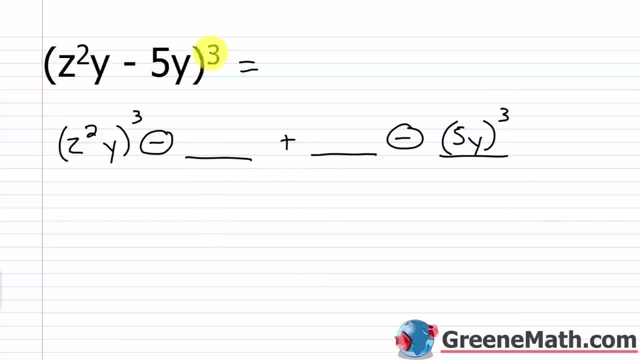 Now, what's gonna be in the middle positions? Well, again, it's the same thing. It's three. remember that exponent is three. So it's three here and three here, And then, in the first instance, you square the first one. 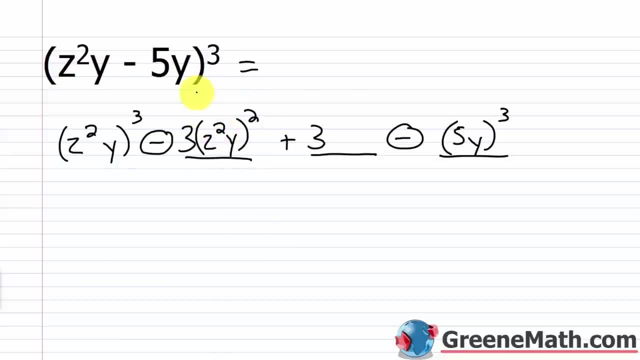 So that's z squared y, that guy squared times, this guy five y. In the second instance you square the second one. So z squared y, Z squared y times. we're gonna do five y squared. I'm kind of running into stuff. 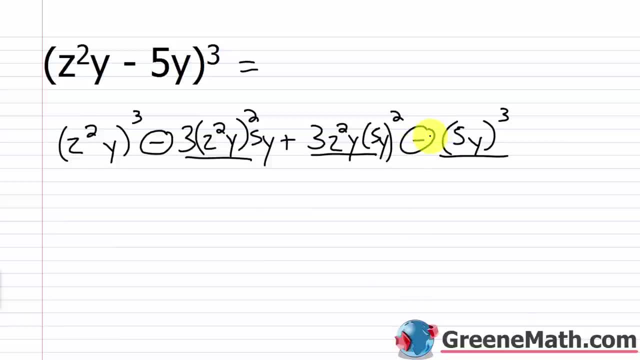 So I know it's. let me kind of scoot this down a little bit And now I can just simplify this. So z squared cubed z stays the same. Two times three is six, Y cubed is just y cubed. 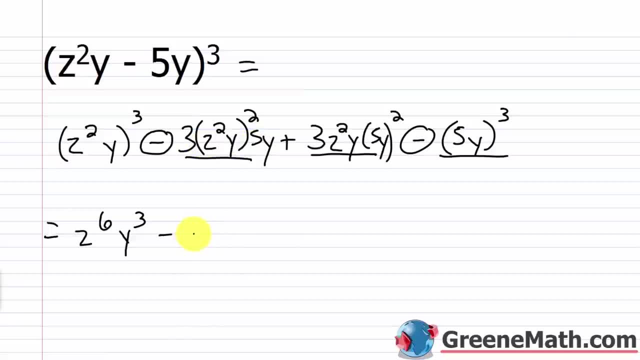 Then minus I have three times five, that's 15.. And then let's think about this: We have z squared, squared, That's z to the fourth power, Then we have y squared, Then we have times y out here. So y squared, times y is y cubed. 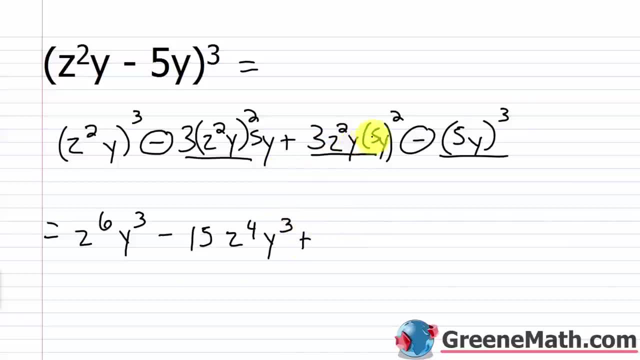 Then plus I have three z squared y. Then we have five y that's squared. So five squared is 25.. 25 times three is 75.. Y squared is y squared, So you'd have z squared y times y squared. 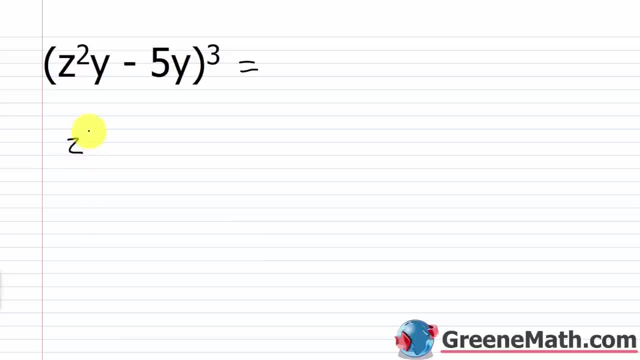 You'll always remember that the first guy is going to be cubed. Now the second term you have a space then plus you have a space then minus. Remember your signs. Before the second term and before the final term. So the final term is this guy right here the 5y cubed. 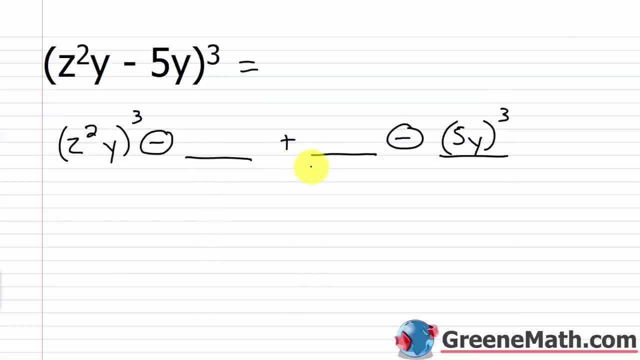 Now what's going to be in the middle positions? Well again it's the same thing. It's 3. Remember that exponent is 3. So it's 3 here and 3 here. And then in the first instance you square the first one. So that's z squared y that guy squared times this guy 5y in the second instance you square the second one. So z squared y times we're going to do 5y squared. I'm kind of running into stuff so I know it's let me kind of scoot this down a little bit. 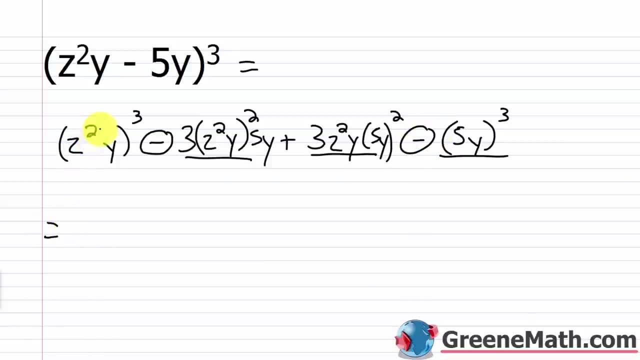 And now I can just simplify this. So z squared cubed z stays the same 2 times 3 is 6 y cubed is just y cubed then minus. I have 3 times 5 that's 15 and then let's think about this. 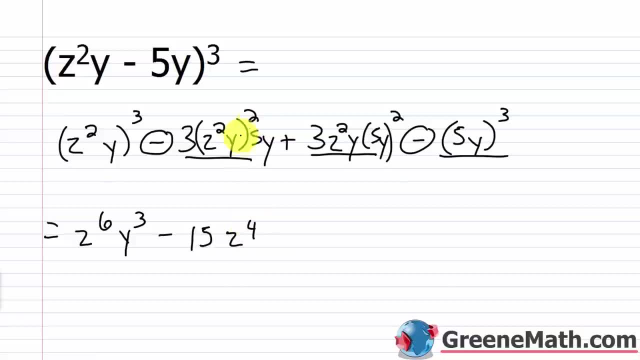 We have z squared squared. That's z to the fourth power. Then we have y squared. Then we have times y out here. So y squared times y is y cubed. Then plus. I have 3 z squared y. Then we have 5y that's squared. So 5 squared is 25. 25 times 3 is 75. y squared is y squared. So you'd have z squared y times y squared. y times y squared is y cubed. 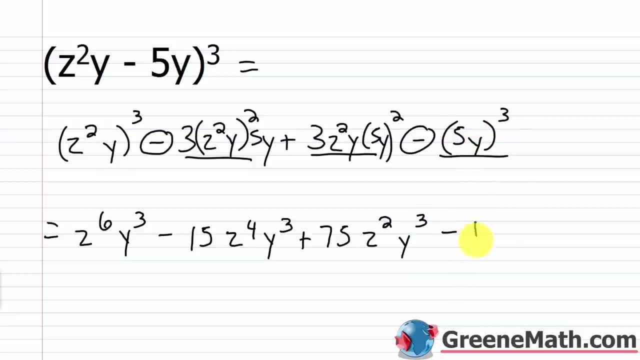 Then minus. Lastly we have 5y cubed. 5 cubed is 125. Then y cubed is just y cubed. So we get z to the sixth power y cubed 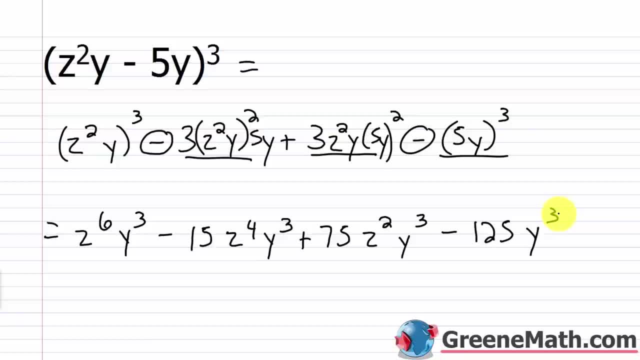 minus 15z to the fourth power y cubed plus 75 z squared y cubed minus 125 y 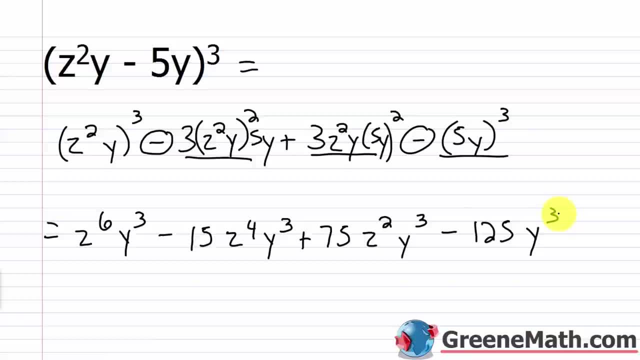 cubed. So this is a perfect example of how much time you would save using this generic formula versus going through and expanding this into z squared y minus 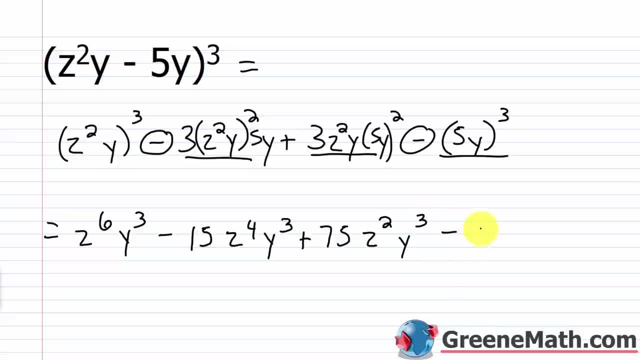 Y times y squared is y cubed, Then minus. lastly we have five y cubed. Five cubed is 125.. Then y cubed is just y cubed. So we get z to the sixth power y cubed, minus 15z to the fourth power y cubed. 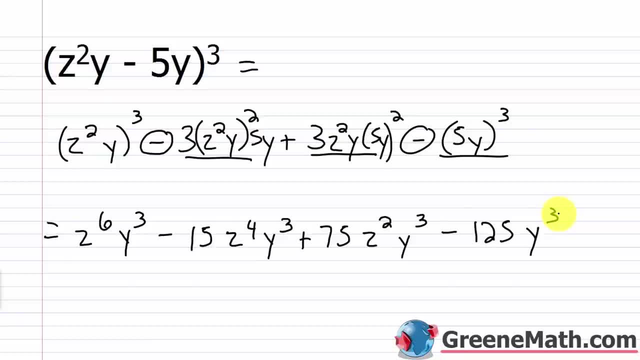 plus 75z squared y cubed minus 125y cubed. So this is a perfect example of how much time you would save using this generic formula versus going through and expanding this into z squared y minus five y times z squared y minus five y. 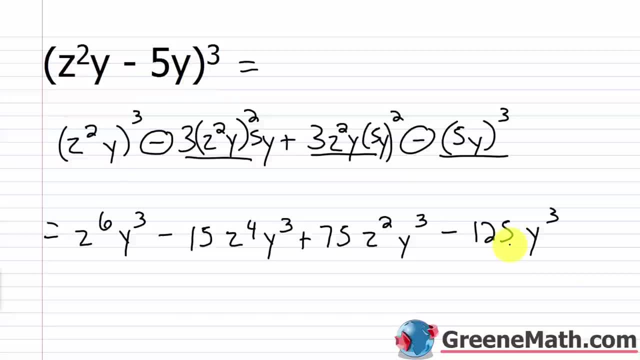 Go ahead and do that and see how long it takes you versus doing it this way, And verify that my answer here is correct. Again: z to the sixth power y cubed minus 15z. to the fourth power y cubed plus 75z squared y cubed minus 125y cubed. 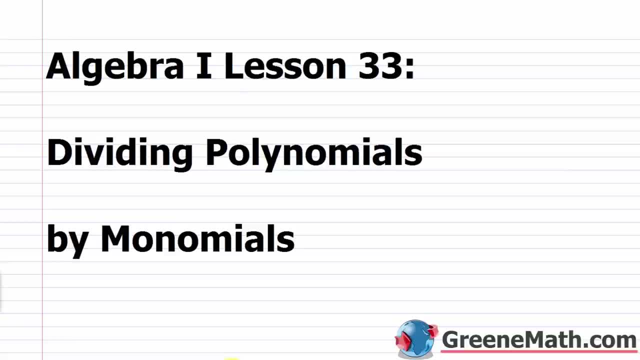 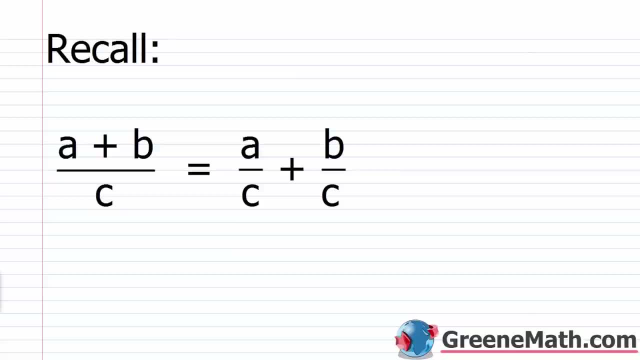 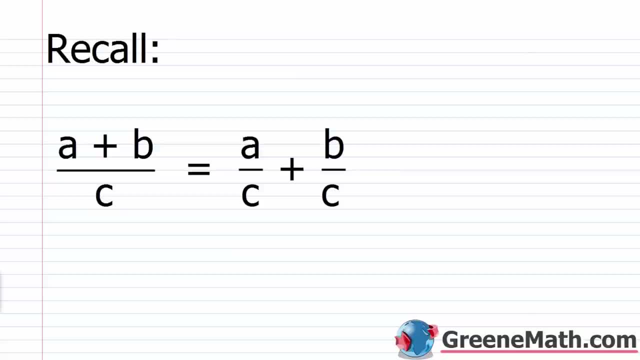 But before we get into the more serious division, we want to start out with something that's very basic, very simple, and that's dividing a polynomial by a monomial. And before we kind of jump into that we need to go over a few things from pre-algebra first. 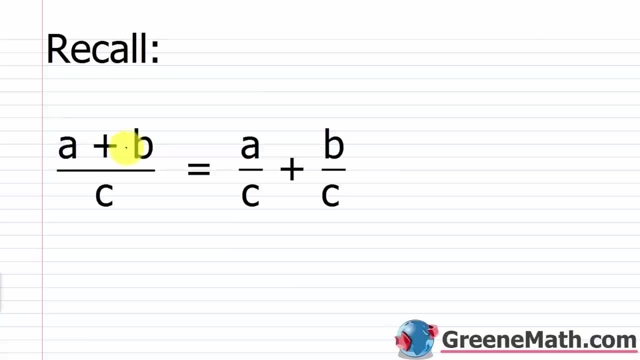 So I want you to recall. if I have something like a plus b, So I want you to recall if I have something like a plus b over c, legally I can write this as a over c plus b over c. These two are the same. 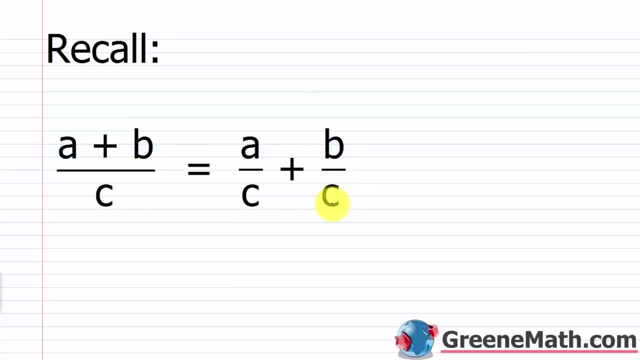 Now, I know in this kind of general form it might not look familiar to you, but all we're saying is that if we have a common denominator- in this case we have a common denominator of c- I can write the sum of the numerators. 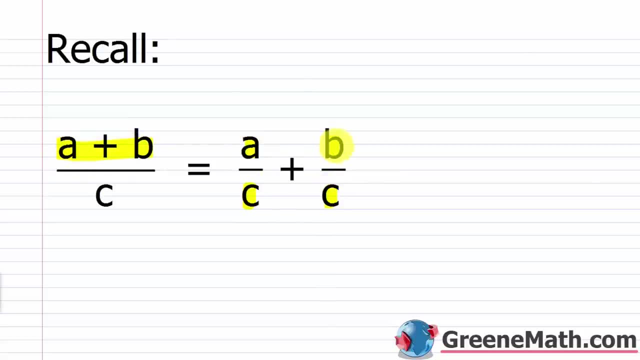 which is a plus b. right, This numerator is a, this numerator is b, so the sum of the numerators over that common denominator of c, As an example with whole numbers. so let's say you saw something like 20 plus four. 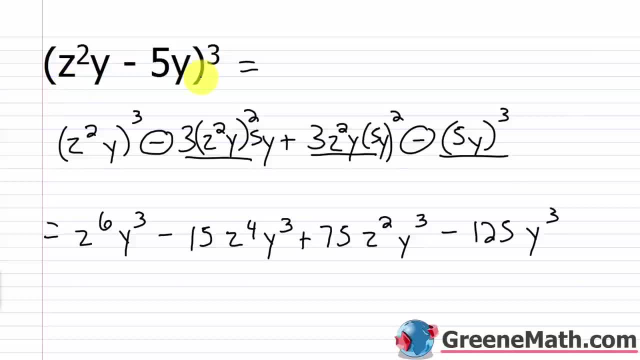 5y times z squared y minus 5y times z squared y minus 5y. Go ahead and do that and see how long it takes you versus doing it this way and verify that my answer here is correct. Again, z to the sixth power y cubed minus 15z to the fourth power y cubed plus 75z squared y cubed minus 125y cubed. Hello and welcome to Algebra 1 Lesson 33. 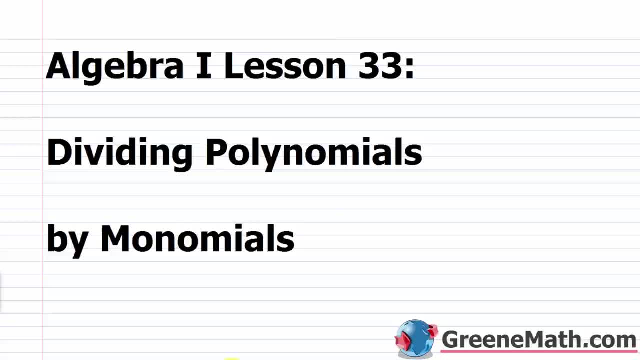 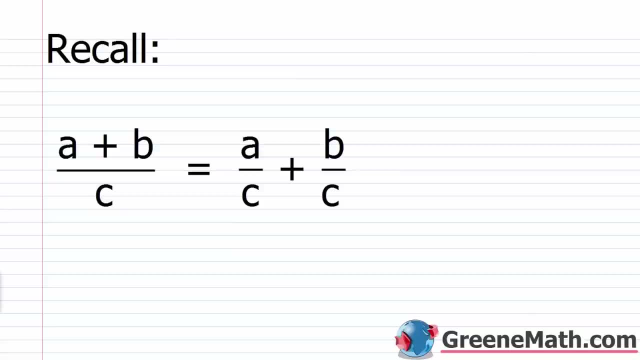 In this video we're going to learn about dividing polynomials by monomials. So far we've learned how to add and subtract with polynomials and we've learned how to multiply polynomials. Now the next logical step is for us to learn how to divide polynomials. But before we get into the more serious division we want to start out with something that's very basic, very simple and that's dividing a polynomial by a monomial. 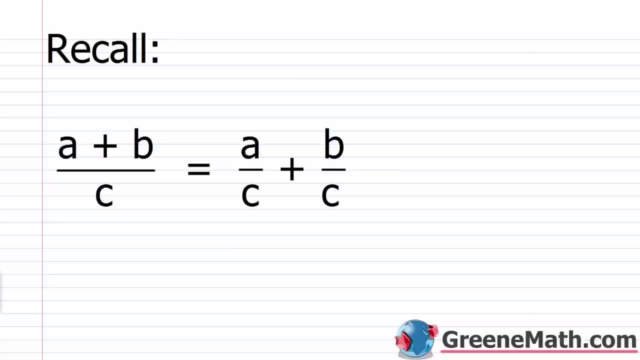 And before we kind of jump into that, we need to go over a few things from pre-algebra first. 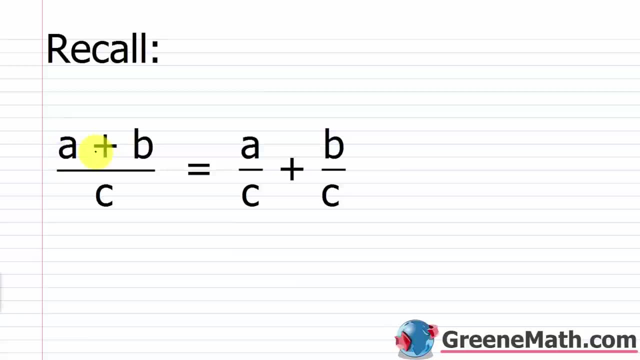 So I want you to recall if I have something like a plus 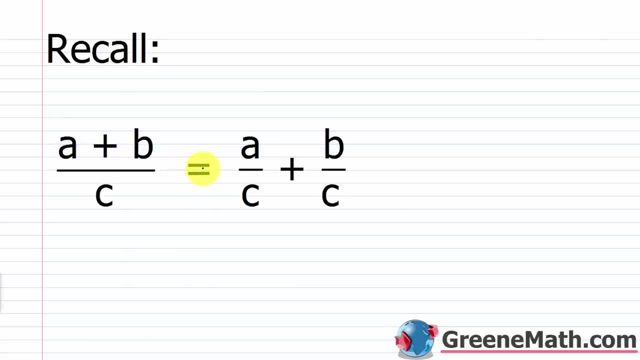 b over c legally I can write this as a over c plus b over c. These two are 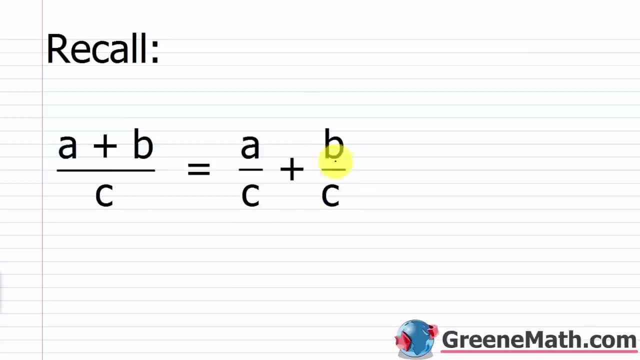 the same. Now I know in this kind of general form it might not look familiar to you, but all 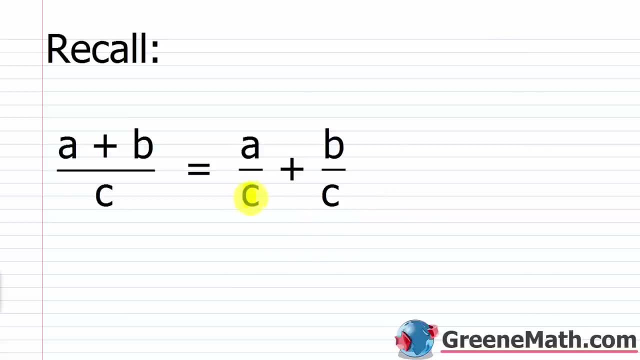 we're saying is that if we have a common denominator in this case we have a common denominator of c, I can write the 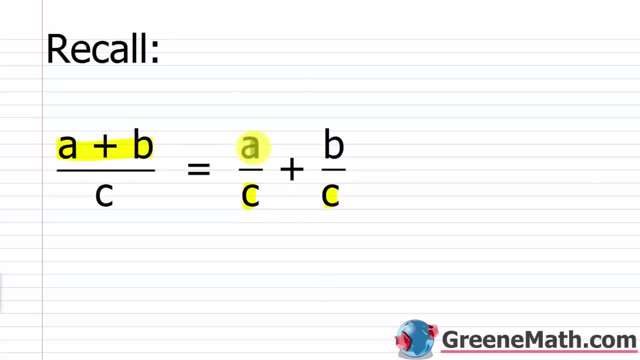 sum of the numerators, which is a plus b. This numerator is a this numerator is b, so the sum of the numerators over that common denominator of c. 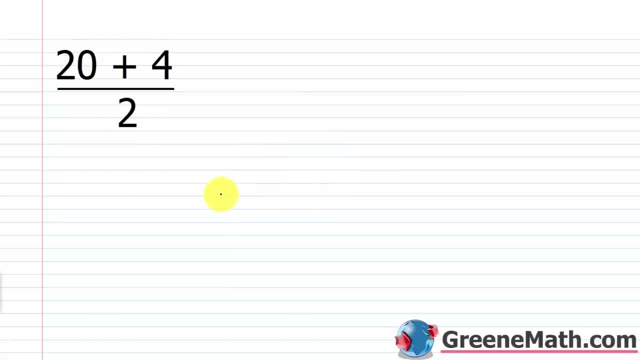 As an example with whole numbers, so let's say you saw something like 20 plus 4 and this is over 2. 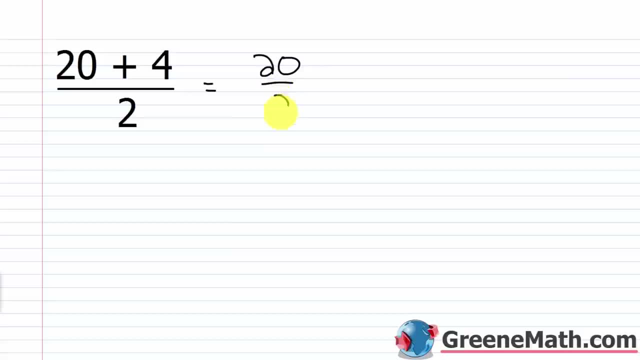 Well I can legally split this up into 20 over 2 plus 4 over 2. And we can see that we get the same answer either way. If I just evaluated this, 20 plus 4 is 24. If I divide it by 2 I get 12. If I do it this way 20 over 2 is 10, 4 over 2 is 2, so 10 plus 2 is 12 also. 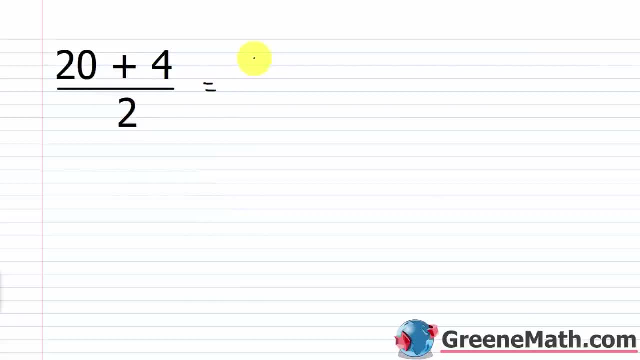 and this is over two. Well, I can legally split this up into 20 over two plus four over two, And we can see that we get the same answer either way. If I just evaluated this, 20 plus four is 24.. 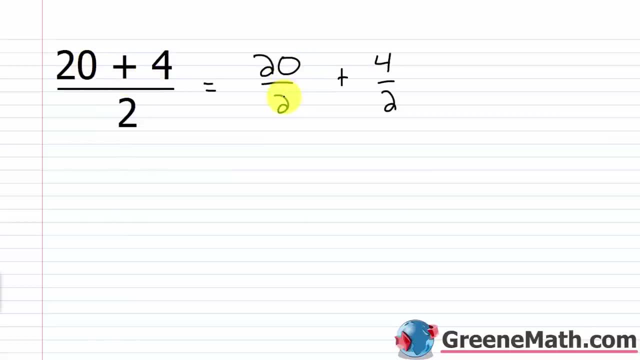 If I divide it by two, I get 12.. If I do it this way, 20 over two is 10,, four over two is two. so 10 plus two is 12. also, And what you're used to seeing is you're used to seeing this. 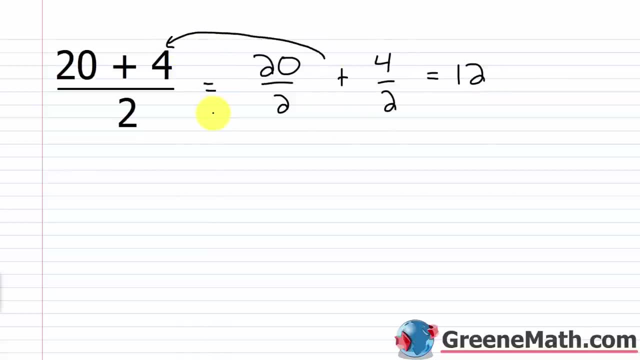 and going to this. And all I'm saying is that it's the same. either way, I can start out kind of in this format and go to this format, And that's what we're gonna need to do in this lesson. So, as another example, let's say you saw something like 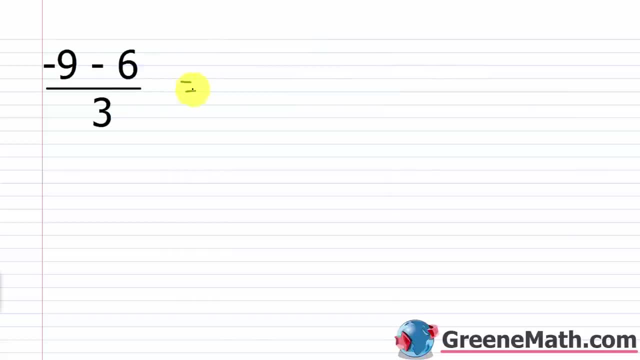 negative nine minus six over three. Again, I can split this up and say I have negative nine over three plus negative six over three. This is just a common denominator here of three, And I could just go back and forth between these two. 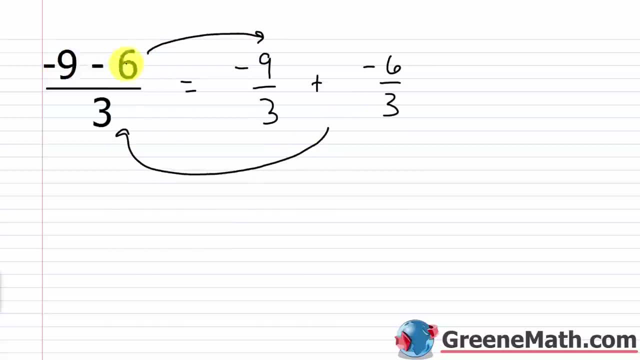 These are the same. And again to kind of prove that if I take negative nine and I subtract away six, I get negative 15.. Then negative 15 divided by three would be negative five. If I kind of do it this way, 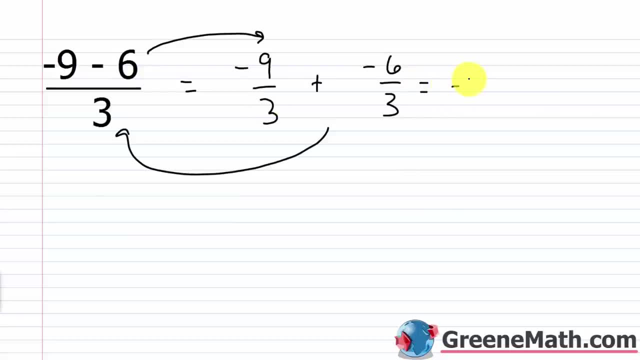 negative nine over three is negative three, And then negative six over three is negative two. So you would have negative three minus two, which again is negative five. So either way, it's the same result. All right. so now that we have that little fun fact. 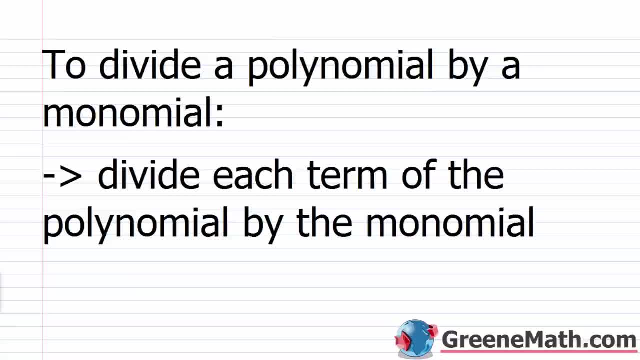 under our belt. we're gonna cover how to divide a polynomial by a monomial. So remember, a monomial is a polynomial that is one single term. So we're dividing by one single term. So, in other words, the divisor in each case. 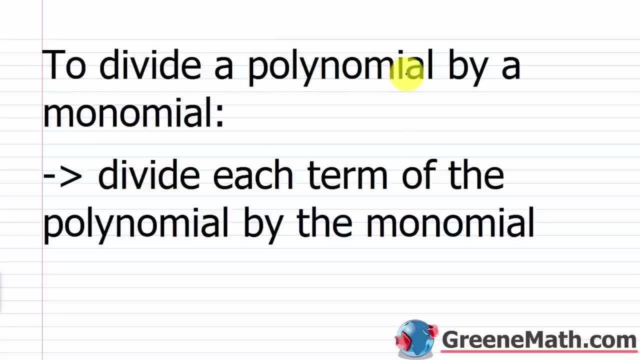 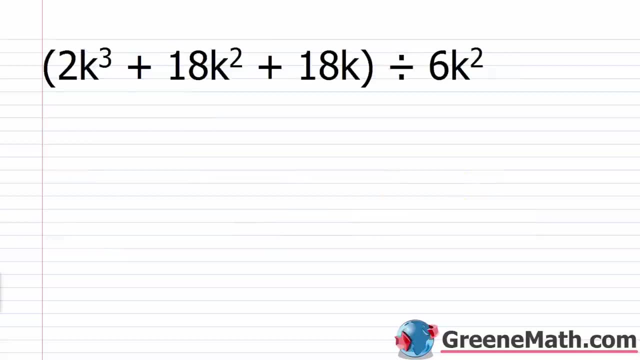 will be a monomial. So to divide a polynomial by a monomial, we want to divide each term of the polynomial by the monomial. We're gonna use the technique we just saw when we looked at those examples with whole numbers. So, starting out with this first one, 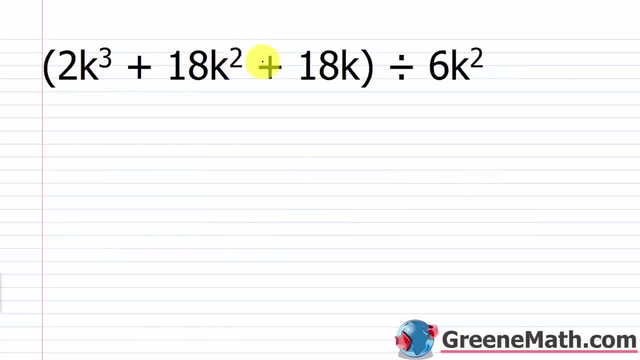 we have 2k cubed plus 18k squared, plus 18k divided by 6k squared. So the first thing I want you to do when you get this problem is set it up as a fraction. So what I'm gonna do is I'm gonna write this as: 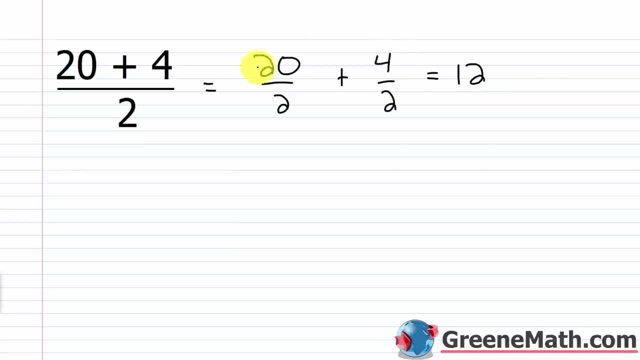 And what you're used to seeing is you're used to seeing this and going to this. And all I'm saying is that it's the same either way. I can start out kind of in this format and go to this format. And that's what we're going to need to do in this lesson. 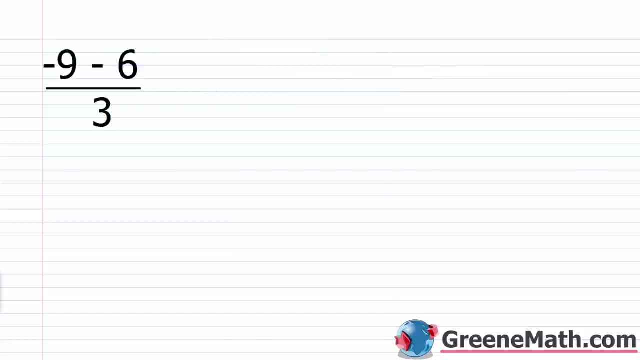 So as another example let's say you saw something like negative 9 minus 6 over 3. 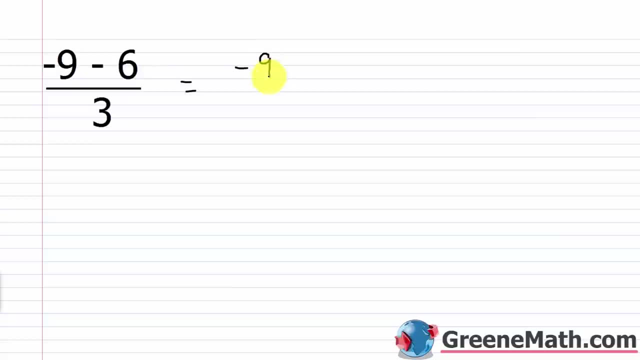 Again I can split this up and say I have negative 9 over 3 plus negative 6 over 3. This is just a common denominator here of 3 and I can just go back and forth between these two. 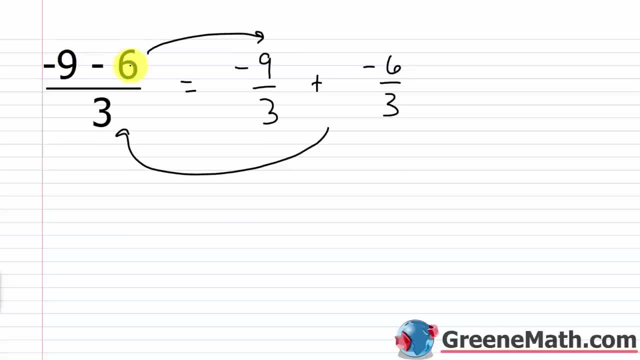 These are the same. And again to kind of prove that if I take negative 9 and I subtract away 6, I get negative 15. 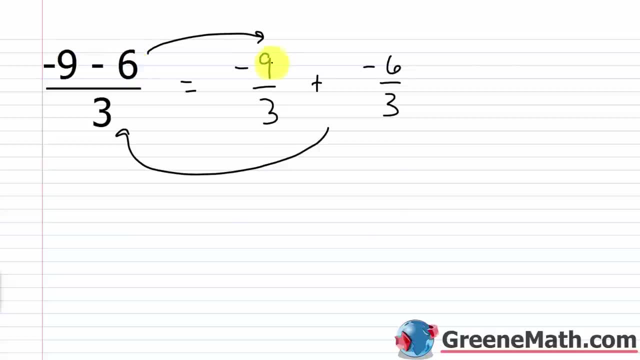 Then negative 15 divided by 3 would be negative 5. If I kind of do it this way 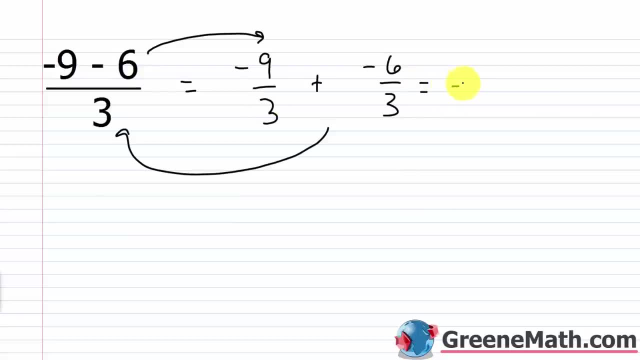 negative 9 over 3 is negative 3 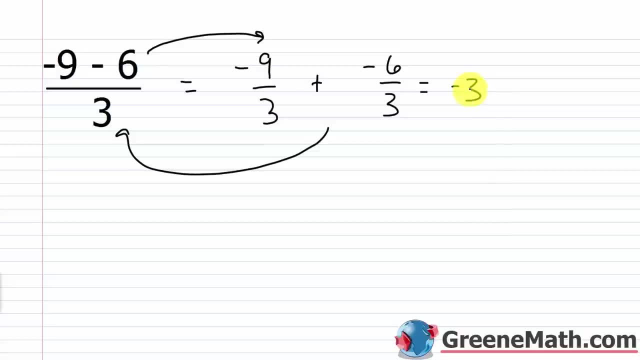 and then negative 6 over 3 is negative 2. 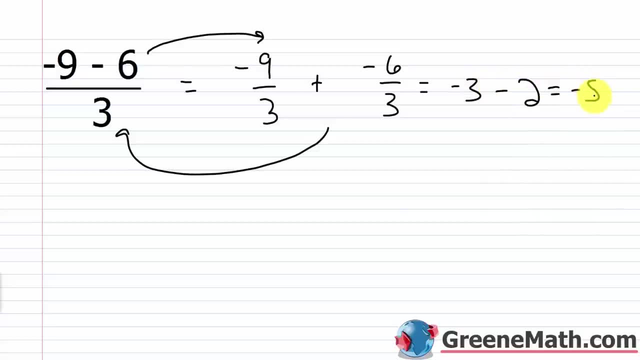 So you would have negative 3 minus 2 which again is negative 5. So either way it's the same result. 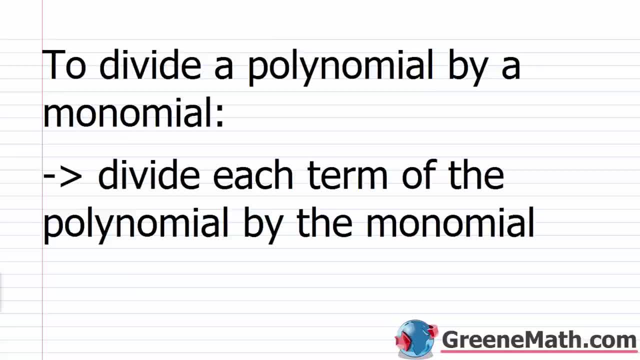 Alright so now that we have that little fun fact under our belt, we're going to cover how to divide a polynomial by a monomial. So remember a monomial is a polynomial that is one single term. So we're dividing by one single term. So in other words the divisor in each case will be a monomial. 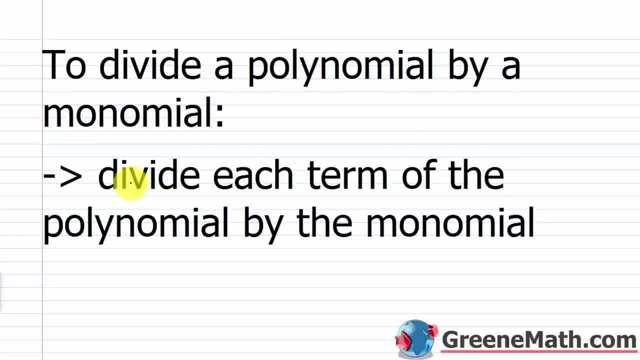 To divide a polynomial by a monomial we want to divide each term of the polynomial by the monomial. 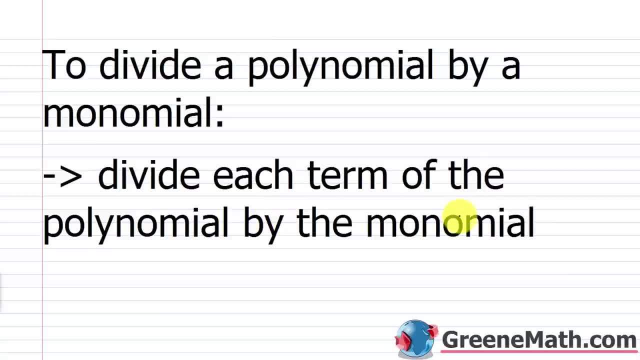 We're going to use the technique we just saw when we looked at those examples with whole numbers. So starting out with this first one 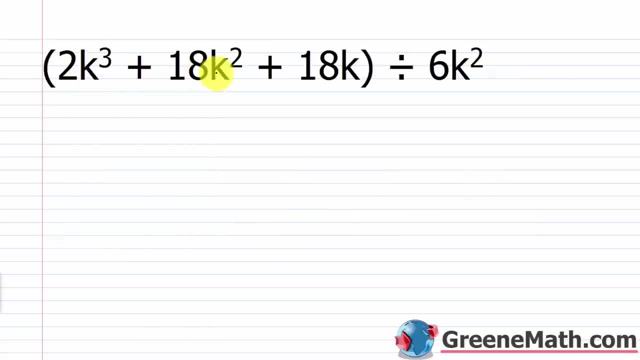 we have 2k cubed plus 18k squared plus 18k divided by 6k squared. 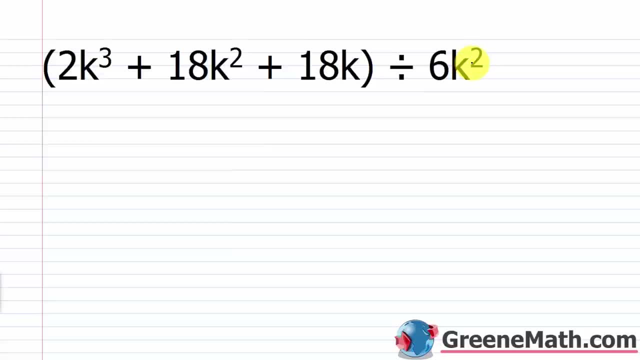 So the first thing I want you to do when you get this problem is set it up as a fraction. So what I'm going to do is I'm going to write this as 2k cubed plus 18k squared plus 18k and then I'm going to put a fraction bar and then my divisor is going to go as the denominator. 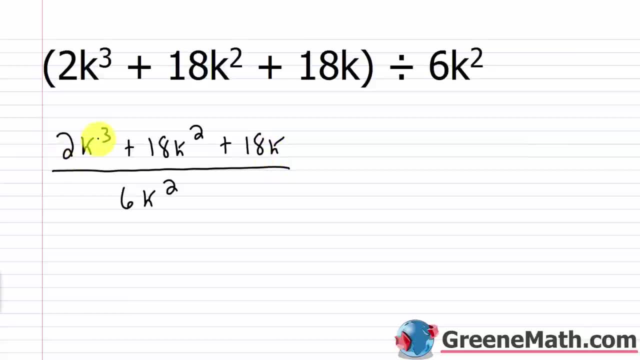 So I have my numerator or my dividend which is 2k cubed plus 18k squared plus 18k and then it's divided by 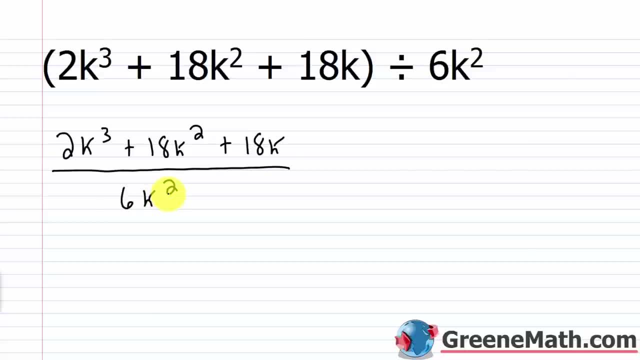 we have our divisor or the denominator 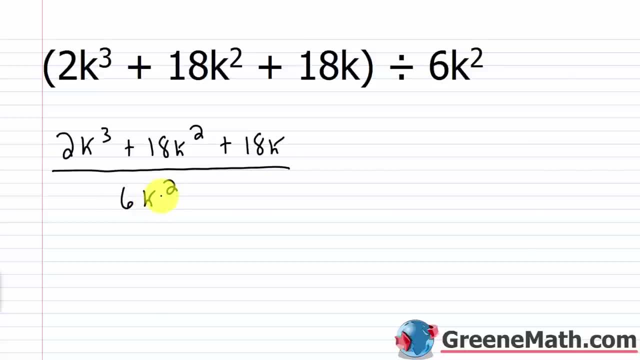 6k squared. So in order to set this problem up it's very very simple. 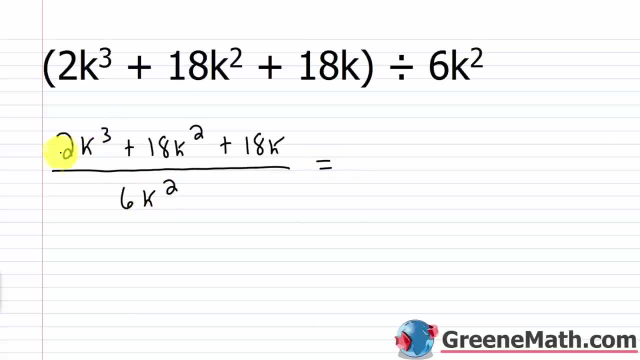 Again, I'm just going to split it up into each term of this polynomial up here in the numerator divided by this monomial down here in the denominator. It's just that simple. 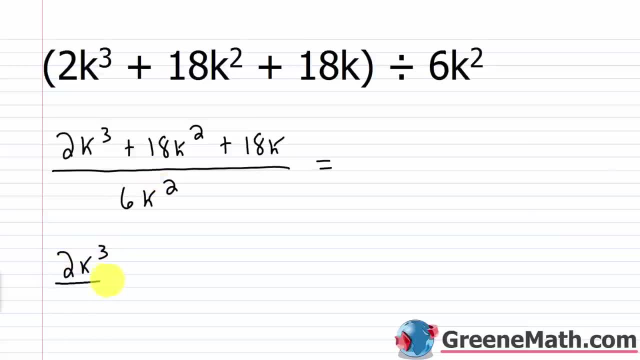 So I would say I have 2k cubed over 6k squared plus, next I have 18k squared 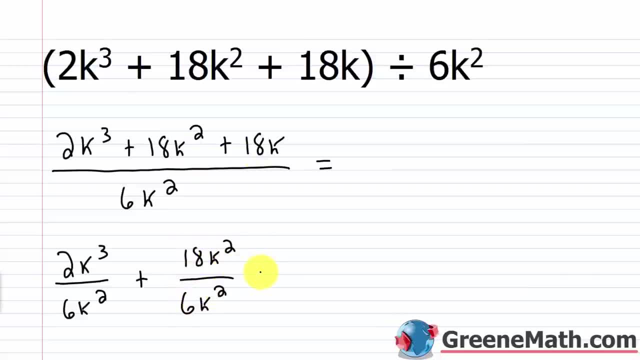 over 6k squared then next I have plus 18k over 6k squared. 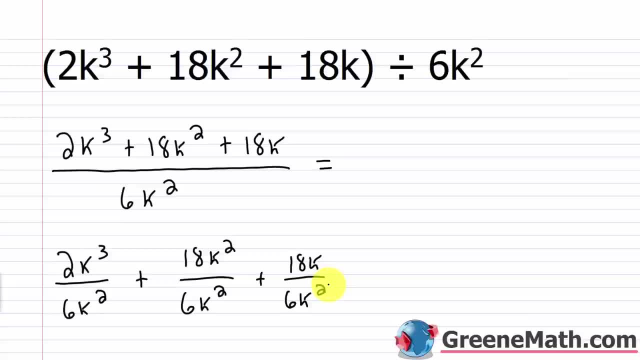 And again, this is perfectly mathematically legal. I have a common denominator here of 6k squared. So I could go right back and write it this with the sum of the numerators 2k cubed plus 18k squared plus 18k over that single common denominator. 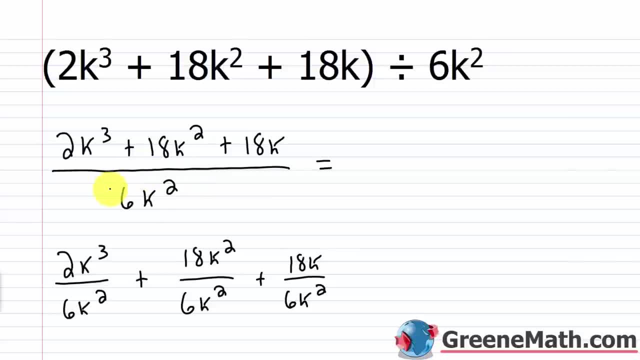 So it's perfectly legal to go back and forth. So once we have set it up in this format all we want to do is simplify each part separately. 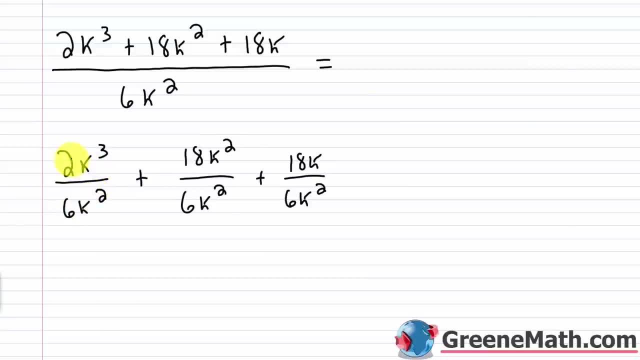 So in other words, I'm going to go through starting here and say, okay if I have 2 over 6, I know I can cancel a common factor of 2 so this is going to cancel and be 1 this is going to cancel and be 3 6 divided by 2 is 3 and then k cubed over k squared 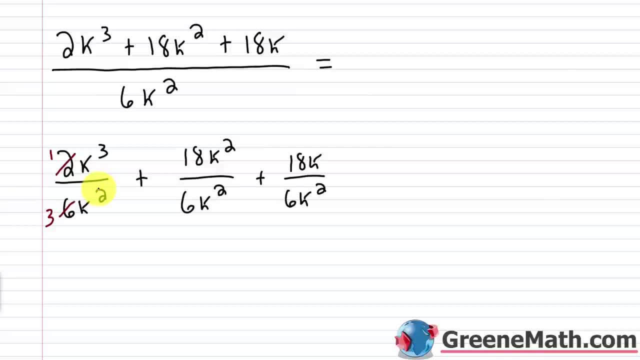 we know that that would be k raised to the power of 3 minus 2. 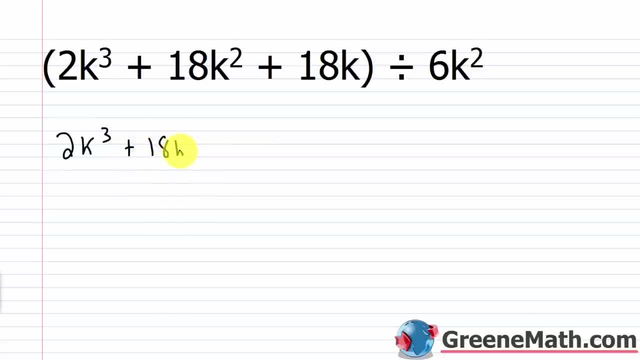 2k cubed plus 18k, squared plus 18k, and then I'm gonna put a fraction bar and then my divisor's gonna go as the denominator. So I have my numerator, or my dividend, which is 2k cubed plus 18k, squared plus 18k. 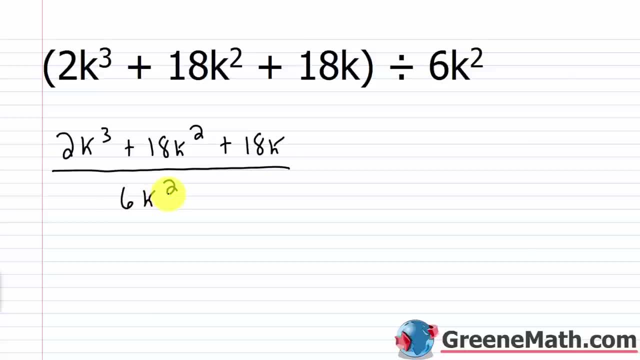 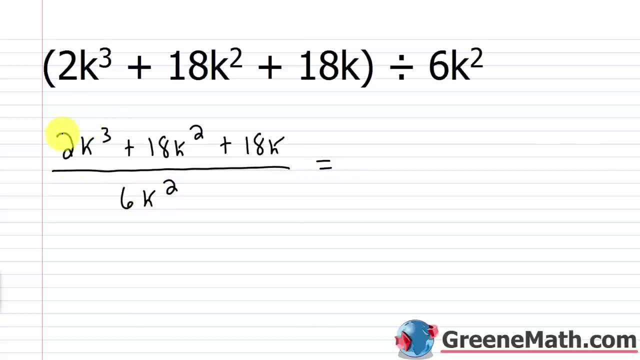 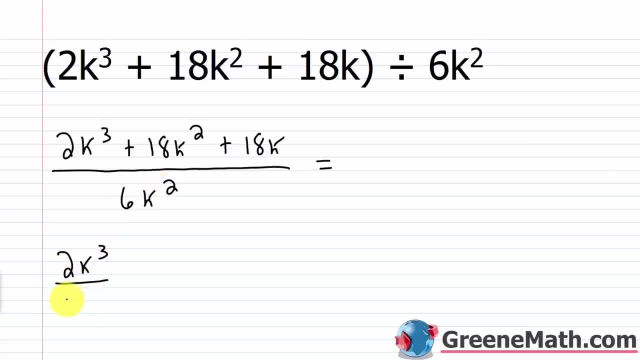 So I would say I have 2k cubed over 6k squared, plus next I have 18k squared over 6k squared, Then next I have plus 18k over 6k squared, And again, this is perfectly mathematical. 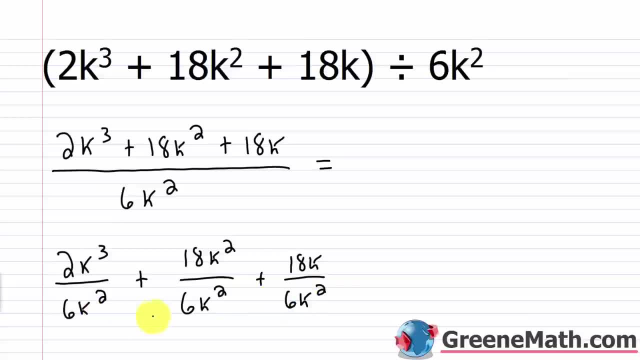 And again, this is perfectly mathematical. I have a common denominator here of 6k squared, So I could go right back and write it this with the sum of the numerators 2k cubed plus 18k squared plus 18k. 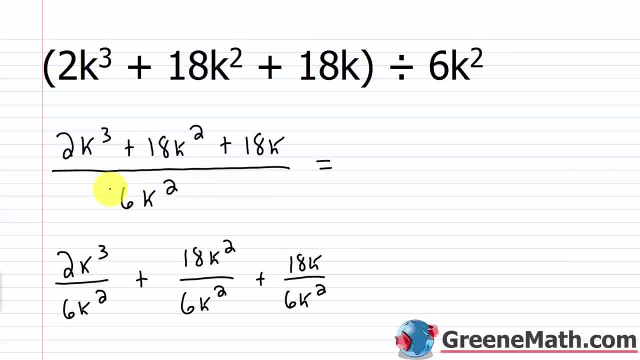 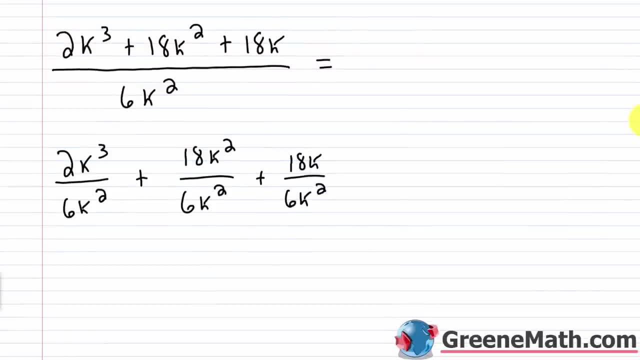 over that single common denominator. So it's perfectly legal to go back and forth. So once we have set it up in this format, all we want to do is simplify each part separately. So, in other words, I'm going to go through, starting here. 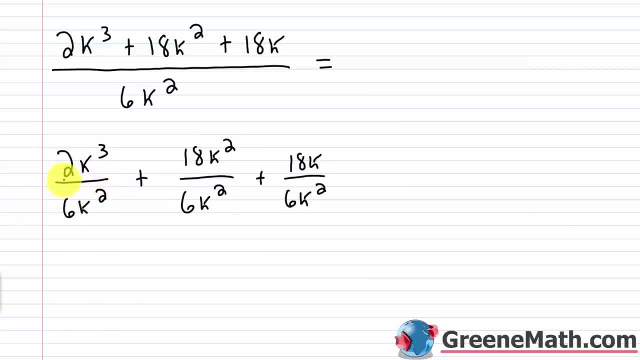 and say, okay, if I have two or three. okay, Okay, if I have two or three, I'm going to go through starting here and say okay, I'm going to go through starting here and say okay, If I have 2 over 6, I know I can cancel a common factor of 2.. 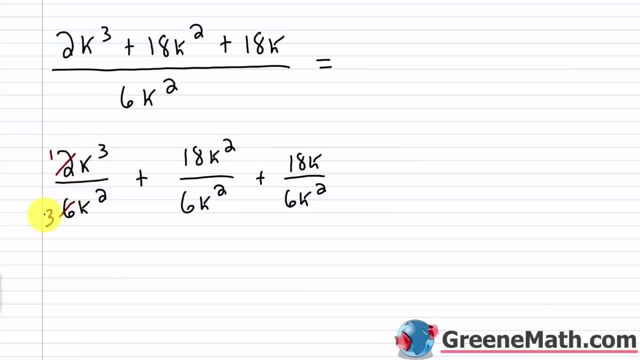 So this is going to cancel and be 1.. This is going to cancel and be 3, right 6 divided by 2 is 3.. And then k cubed over k squared, we know that that would be k raised to the power of 3 minus 2.. 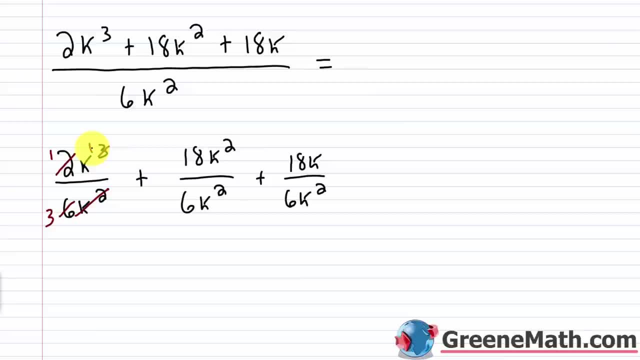 So this is going to cancel and this is going to be a 1, right. So that's k to the first power. So let's go ahead and put equals and then we'll write the results as we go. So this is k to the first power, or just k over, just a 3 in the denominator. 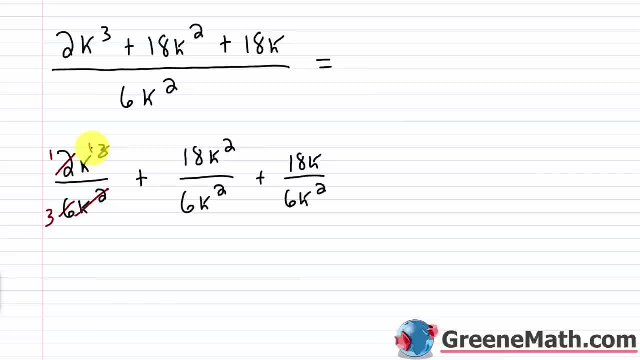 So this is going to cancel and this is going to be a 1. So that's k to the first power. So let's go ahead and put equals and we'll write the results as we go. 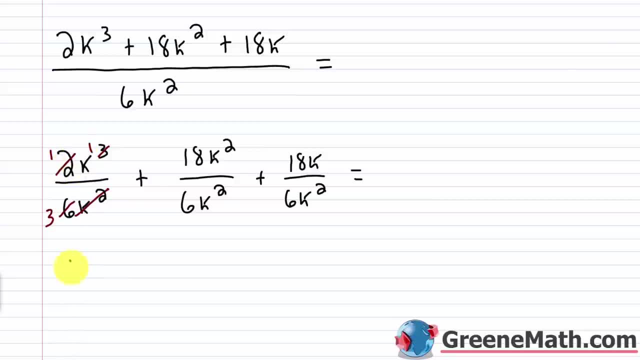 So this is k to the first power, or just k 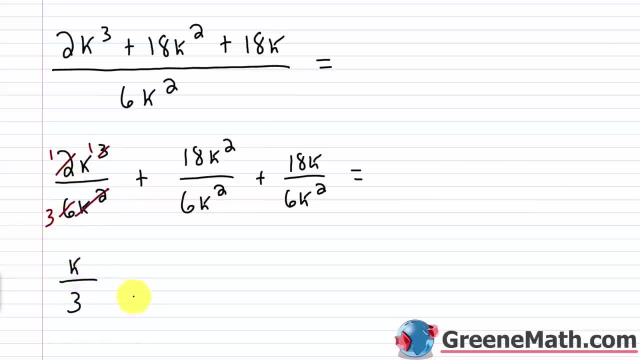 over just a 3 in the denominator and then plus, if I look at this 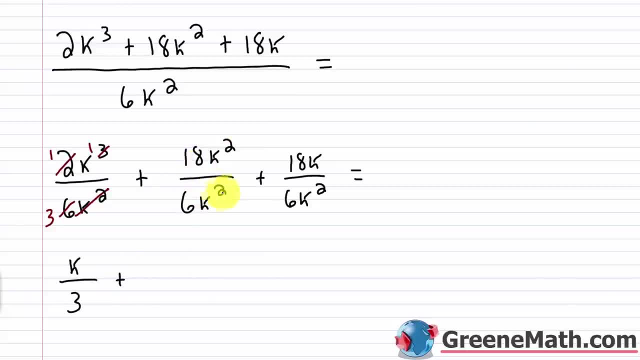 right here, I have 18 k squared over 6k squared Well 18 divided by 6 is 3. k squared 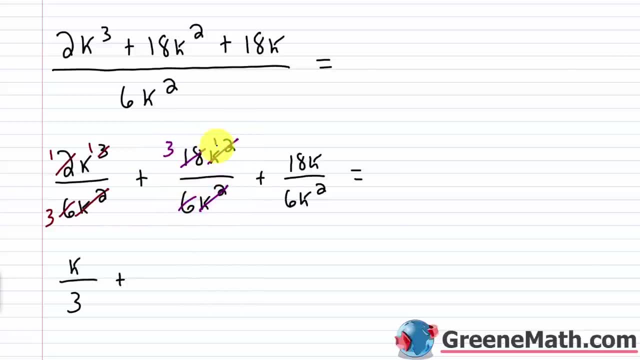 over k squared is 1. So this is going to cancel completely. That's going to be 1 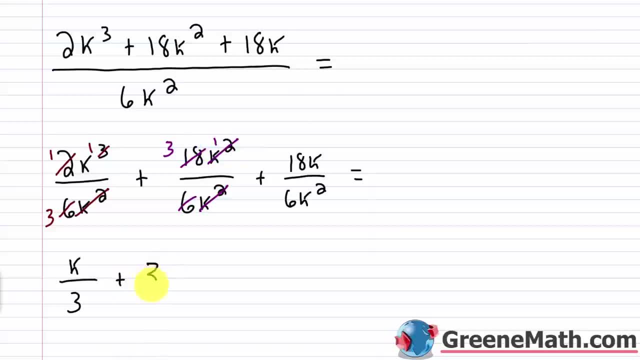 So then plus, I'm going to put a 3 here and then lastly I have plus 18k over 6k squared So 18 divided by 6 again is 3. k over k squared So this is k to the first power So remember if you use your quotient rule for exponents this is going to be k to the power of 1 minus 2 or k to the power of negative 1. k to the power of negative 1 is what? It's 1 over k So essentially just eyeballing that you can see that this cancels out 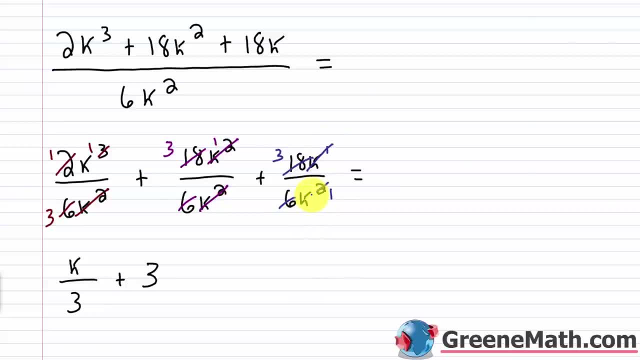 with one of the factors of k here You just have a k to the first power in the denominator So this would be plus 3 over k to the first power or just 3 over k So this is your answer You get k over 3 plus 3 plus 3 over k 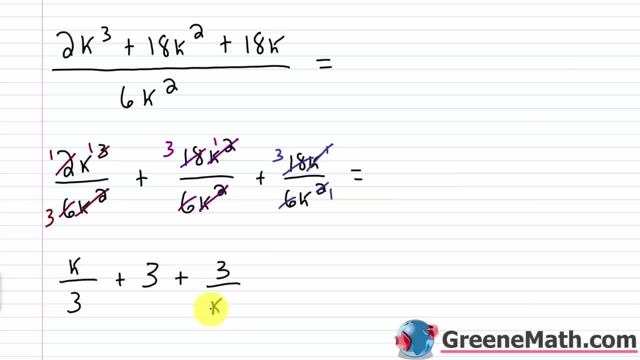 Now, I want you to remember something else from pre-algebra Let me scroll down and get a little room going for this Let's say that I 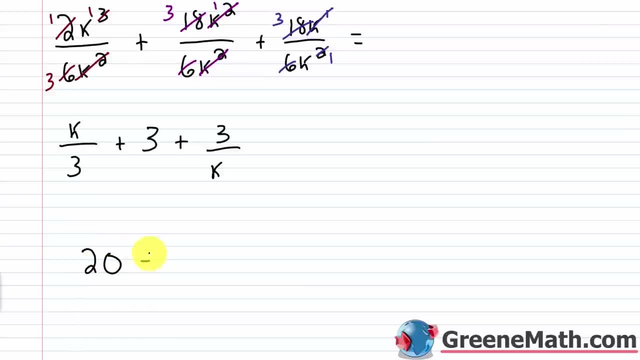 had something like 20 divided by 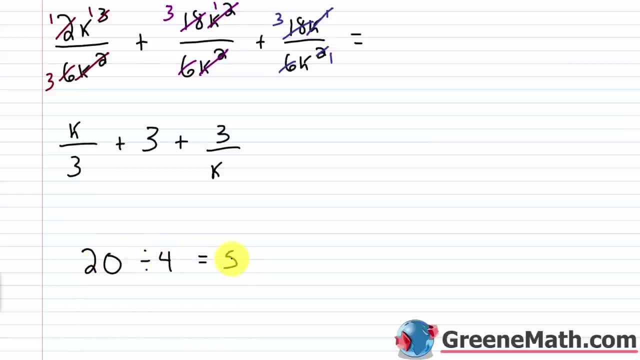 4 and we all know this is 5 So I have my dividend, this is my dividend this is my divisor 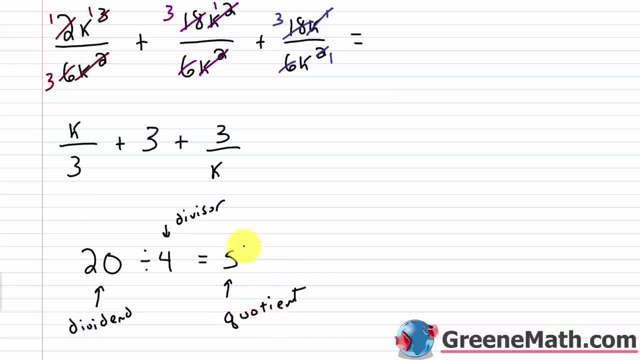 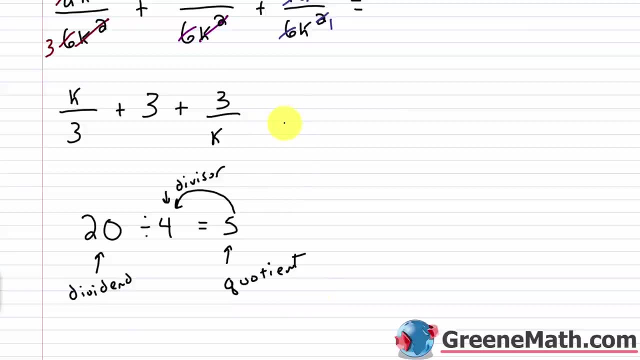 So how can I check the result? Remember, I can go backwards I can take the quotient and multiply it by the divisor and I should get my dividend back. So in this particular case, this is our quotient. So I should be able to multiply this quotient 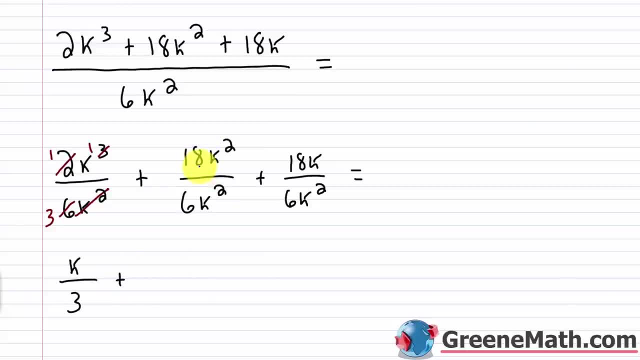 And then plus, if I look at this right here, I have 18k squared over 6k squared. Well, 18 divided by 6 is 3.. k squared over k squared is 1.. So this is going to cancel completely. 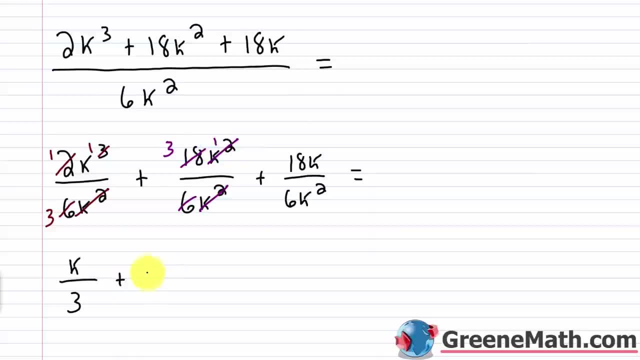 That's going to be 1.. So then plus, I'm going to put a 3 here, And then, lastly, I have plus 18k over 6k squared, So this is going to cancel completely. So 18 divided by 6, again is 3.. 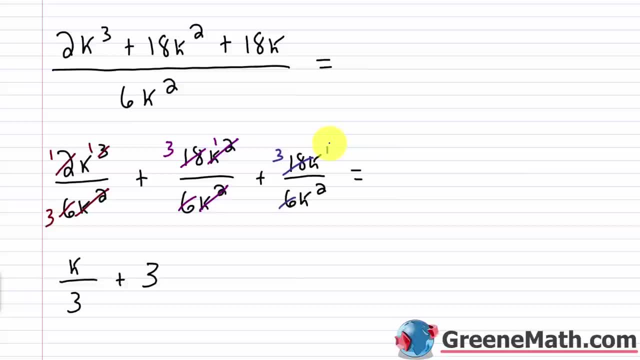 k over k squared, So this is k to the first power. So remember, if you use your quotient rule for exponents, this is going to be k to the power of 1 minus 2, or k to the power of negative 1.. 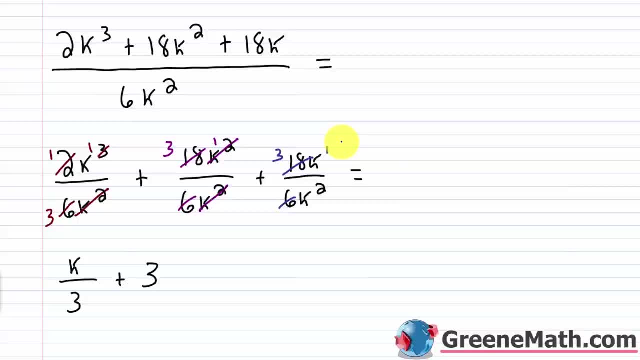 k to the power of negative 1 is what It's: 1 over k, So essentially just eyeballing that you can see that this cancels out with one of the factors of k. here You just have a k to the first power in the denominator. 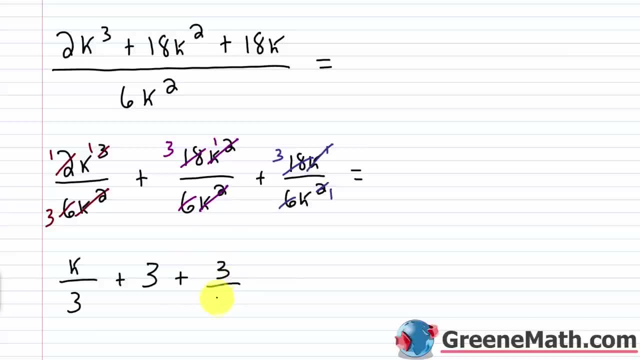 So this would be plus 3 over over k to the first power, or just 3 over k. So this is your answer: You get k over 3, plus 3, plus 3 over k. Now I want you to remember something else from pre-algebra. 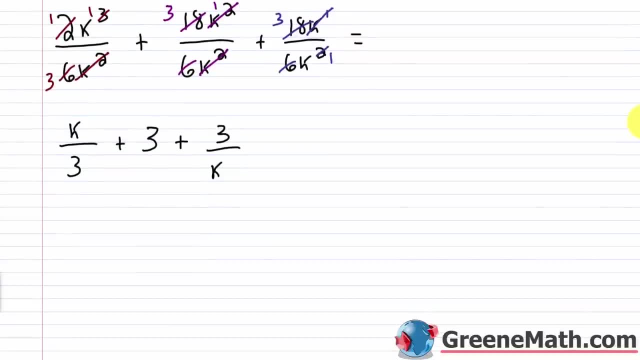 Let me scroll down and get a little room going for this. Let's say that I had something like 20 divided by 4, and we all know this is 5.. So I have my dividend. This is my dividend. This is my divisor. 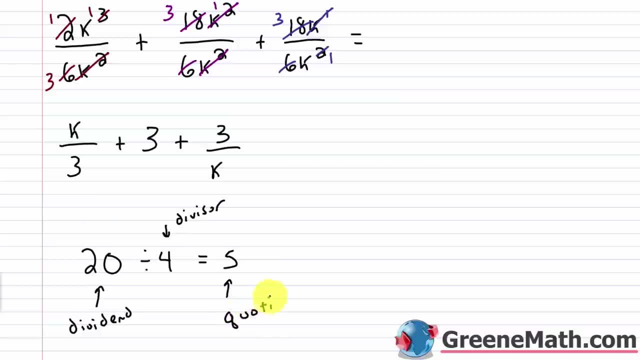 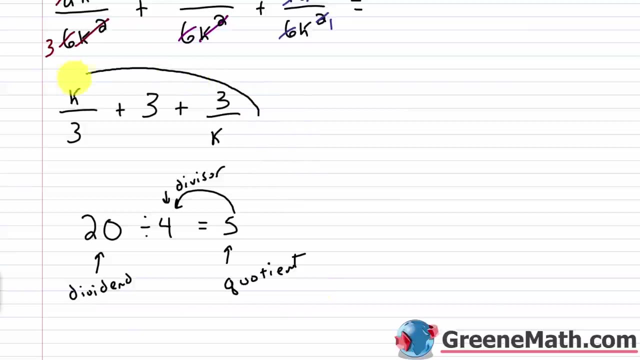 And then this is my quotient. So how can I check the result? Remember, I can go backwards. I can take the quotient and multiply it by the divisor and I should get my dividend back. So, in this particular case, this is our quotient. 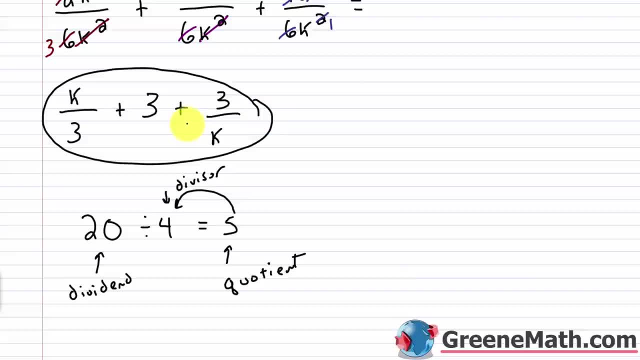 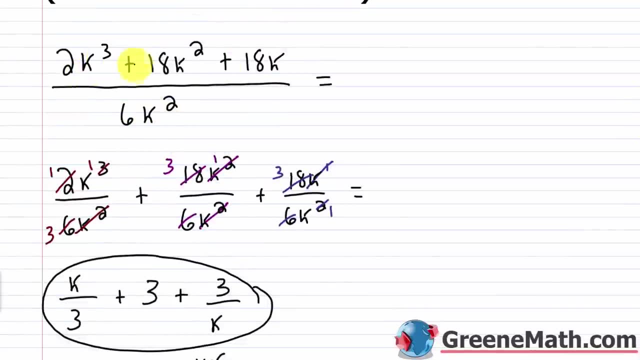 So I should be able to multiply this quotient by our divisor- Remember, the divisor is 6k squared- And then I should get the dividend back, The 2k cubed plus 18k squared plus 18k. So let's check that out. 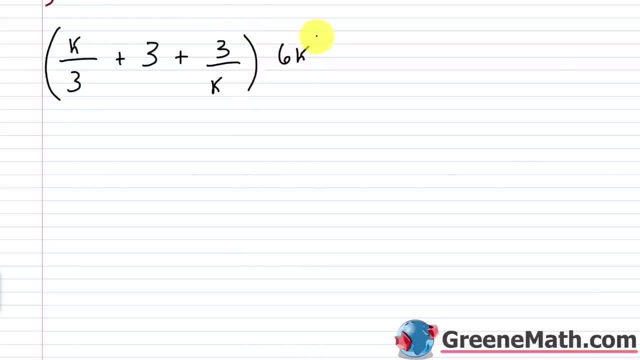 Okay, so I'm going to multiply this guy by 6k squared, And again, all I'm going to use is the distributive property. So 6k squared times k over 3.. Let's just write that out like this: 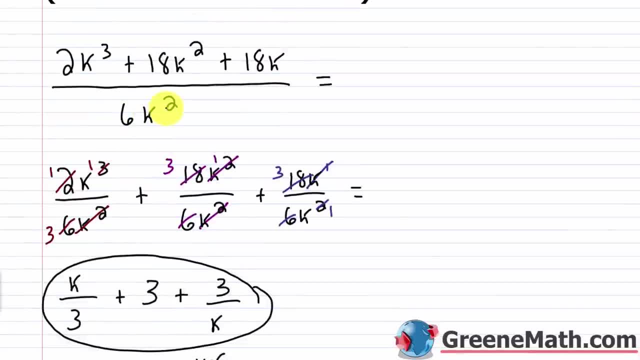 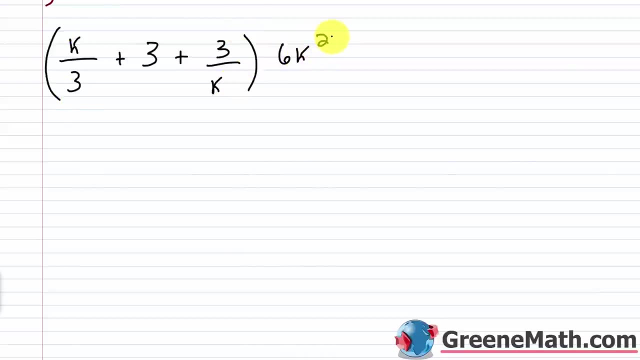 by our divisor Remember, the divisor is 6k squared and then I should get the dividend back. The 2k cubed plus 18k squared plus 18k. So let's check that out. So I'm going to multiply this guy by 6k squared And again, all I'm going to use is the distributive property. So 6k squared times k over 3. Let's just write that out like this. So 6k squared times k over 3 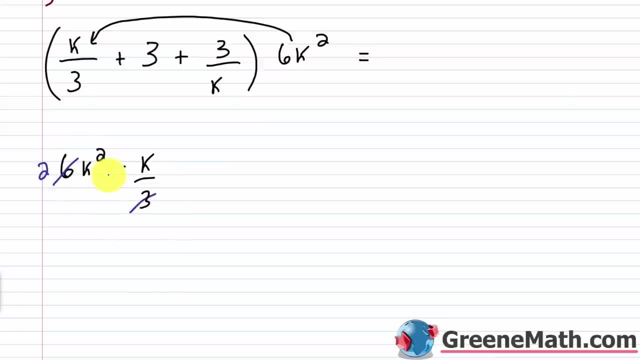 Well, we know that the 6 would cancel with the 3 and give me a 2 And then k squared times k is k cubed 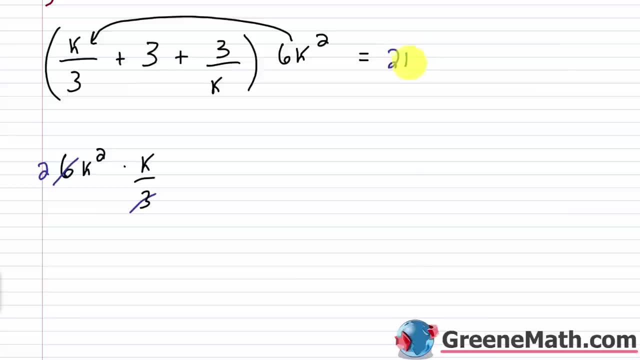 So for the first part I'm going to put 2k cubed 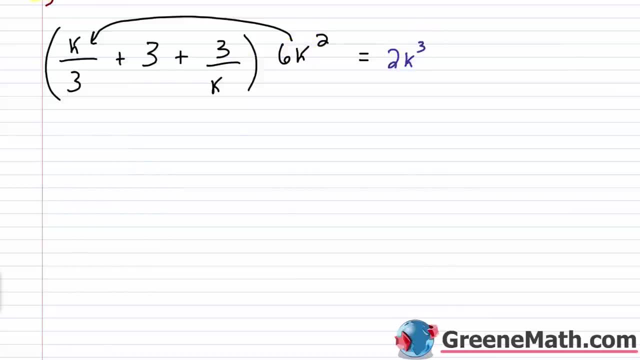 Let me erase this Then we have 6k squared 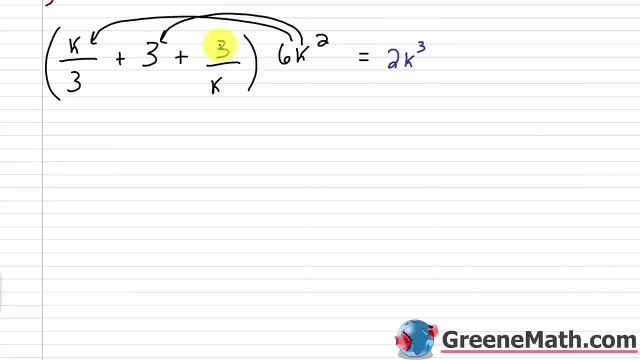 6k squared times 3 Well that's easy. It's just 3 times 6 which is 18 And then k squared comes along 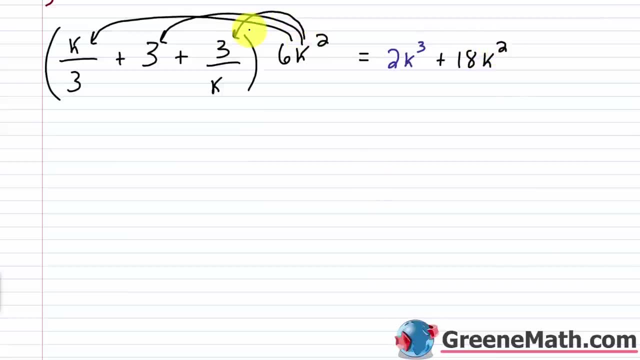 for the ride And then lastly I have 6k squared times 3 over k So 6k 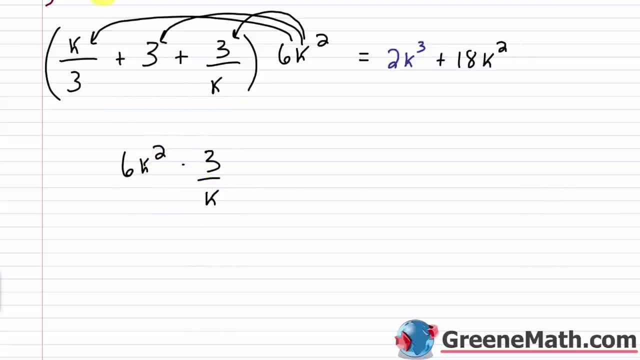 squared times 3 over k Well we can see that one of the factors of k here would cancel with this k And it would have 6 times 3 that's 18 So 18k. So plus 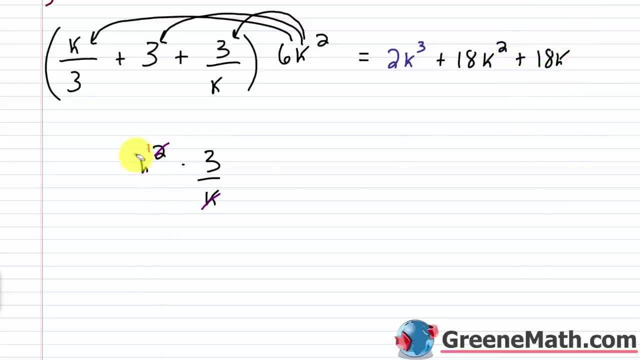 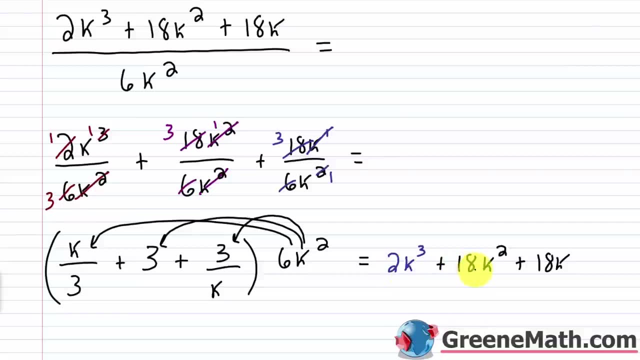 18k So let's see if this was our original dividend So we scroll back up here and we see that it was 2k cubed plus 18k squared plus 18k 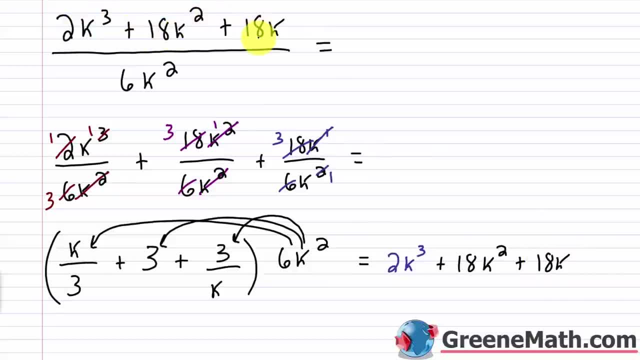 2k cubed plus 18k squared plus 18k So because we multiplied 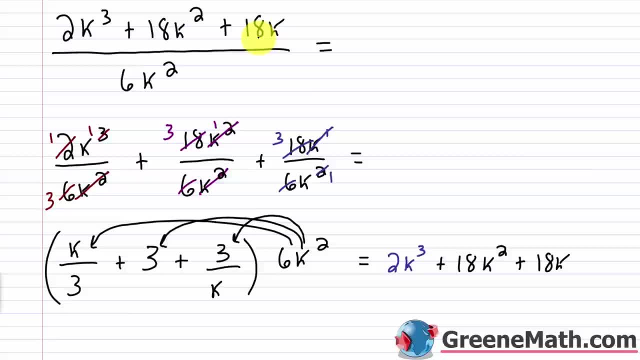 our divisor by the quotient and it gave us the dividend back we know we have the correct answer So it's very important especially when you first start to go back and check your answer make sure that you got the 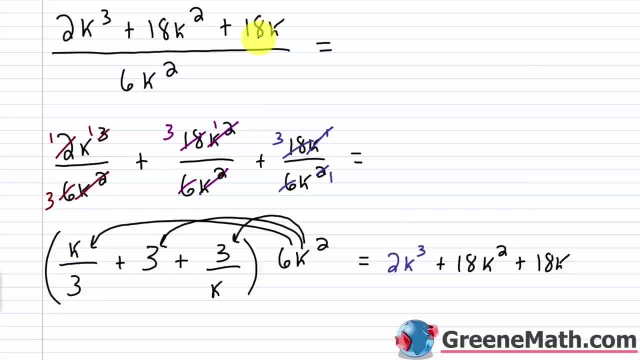 correct one. That way if you didn't you can correct the mistake right away 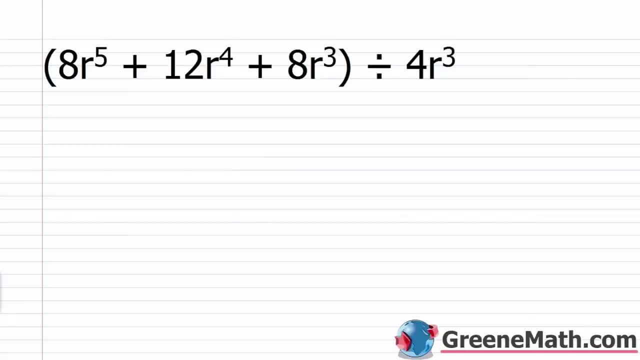 Alright let's take a look at another one So we have 8r to the fifth power plus 12r to the fourth power plus 8r cubed divided by 4r cubed So again I'm going to write this as a fraction. So I'm going to write this 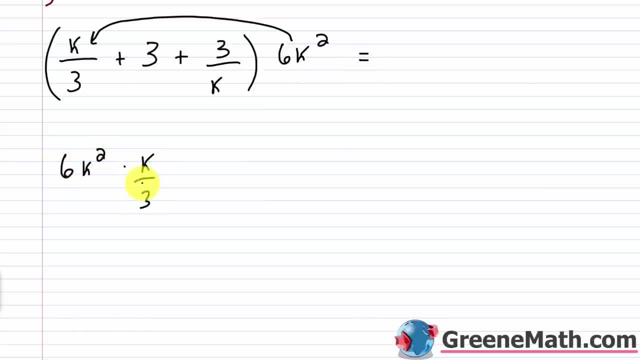 So 6k squared times k over 3.. Well, we know that the 6 would cancel with the 3 and give me a 2. And then k squared times k is k cubed. So for the first part I'm going to put 2k cubed. 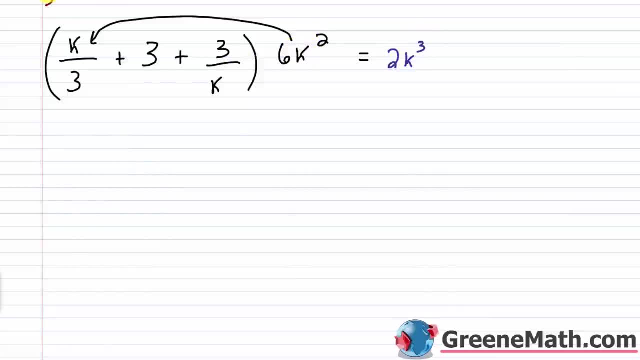 Let me erase this. Then we have 6k squared. 6k squared times 3.. Well, that's easy, It's just 3 times 6,, which is 18.. And then k squared comes along for the ride. 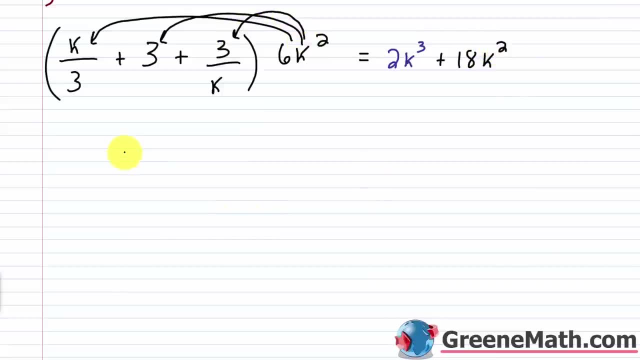 And then, lastly, I have 6k squared times 3 over k. So 6k squared times 3 over k. Well, we can see that One of the factors of k here would cancel with this k And I'd have 6 times 3.. 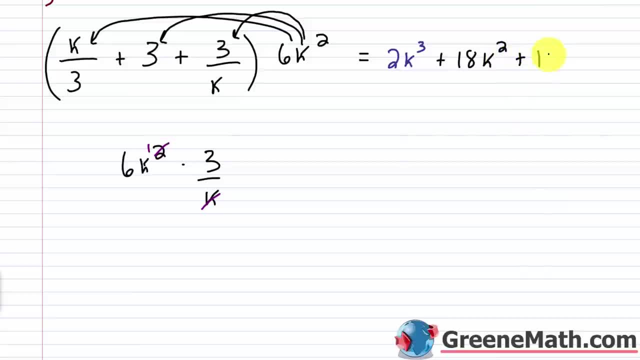 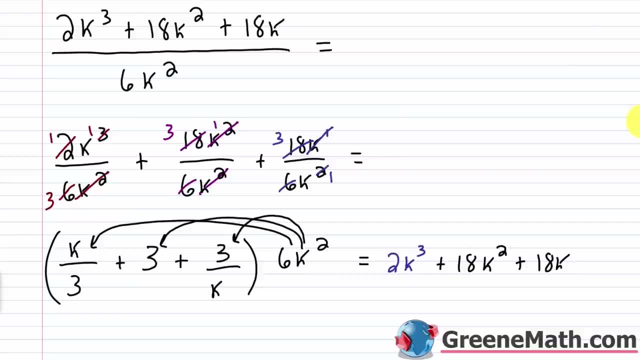 That's 18.. So 18k. So plus 18k. So let's see if this was our original dividend. So we scroll back up here and we see that it was 2k cubed plus 18k, squared plus 18k. 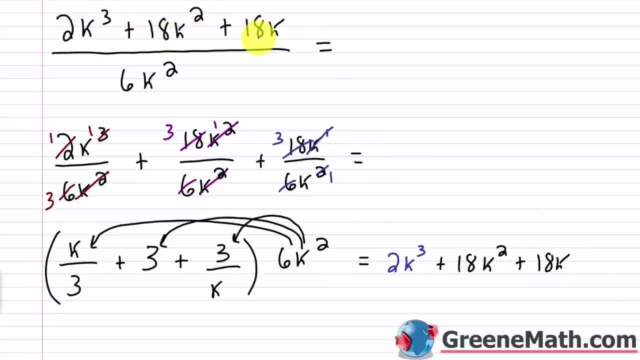 2k cubed plus 18k squared plus 18k. So because we multiplied our divisor by the quotient and it gave us the dividend, we know we have the correct answer. So it's very important, especially when you first start. 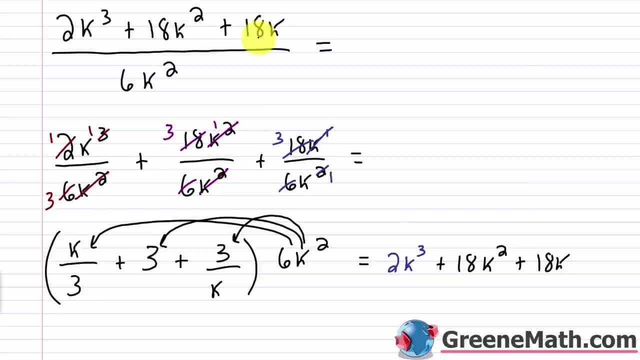 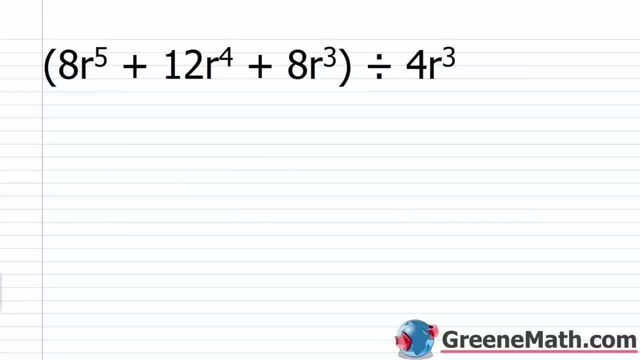 to go back and check your answer. Make sure that you got the correct one. That way, if you didn't, you can correct the mistake right away. All right, let's take a look at another one. So we have 8r to the 5th power plus 12r to the 4th power plus 8r cubed divided by 4r cubed. 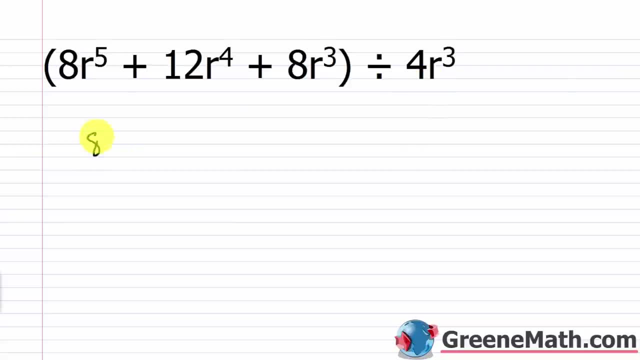 So again, I'm going to write this as a fraction. So I'm going to write this as 8r to the 5th power plus 12r to the 4th power. So I'm going to write this as 8r to the 5th power plus 12r to the 4th power, plus 8r cubed. 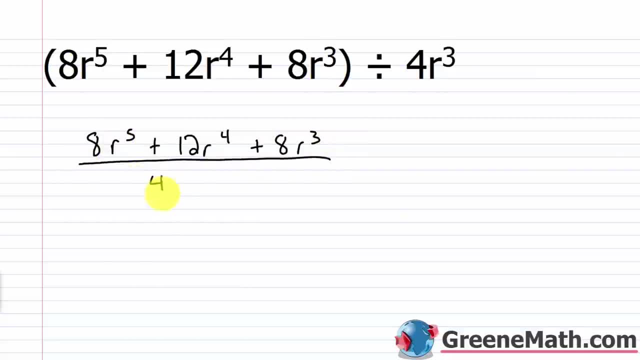 That's the numerator, right? That's the dividend. So then this is divided by 4r- 4r cubed, And then I'm just going to split this up, right? This is just a common denominator. So I'm going to say this is 8r to the 5th power over 4r cubed, plus 12r to the 4th power over 4r cubed. 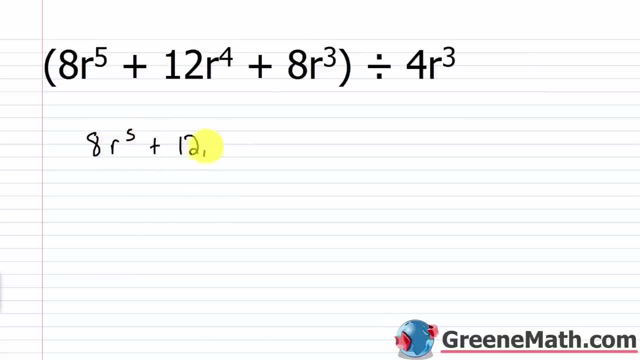 as 8r to the fifth power plus 12r to the fourth power plus 8r cubed That's the numerator That's the dividend 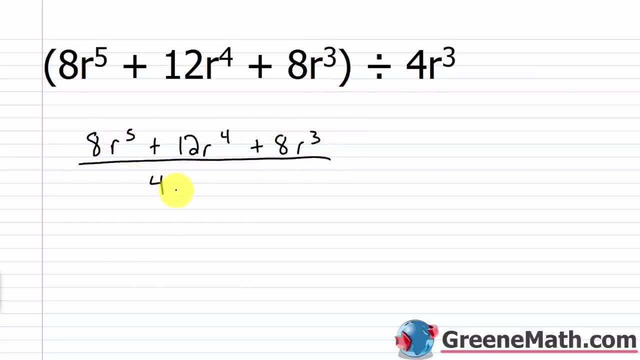 So then this is divided by 4r 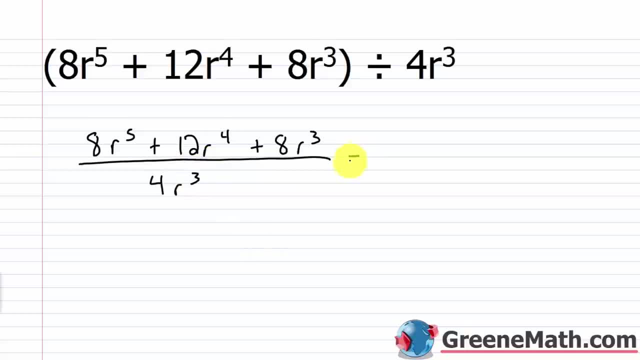 4r cubed And then I'm just going to split this up This is just a common denominator So I'm going to say this is 8r to the fifth power 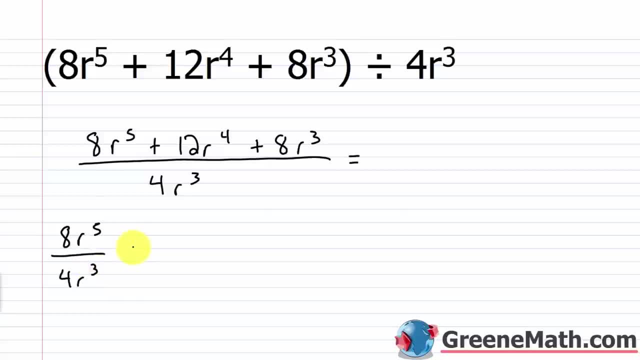 over 4r cubed plus 12r to the fourth power over 4r cubed 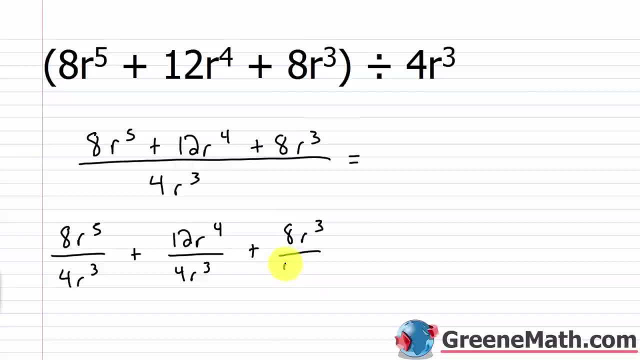 plus 8r cubed over 4r cubed And then once I have it in this format it's very easy to go through 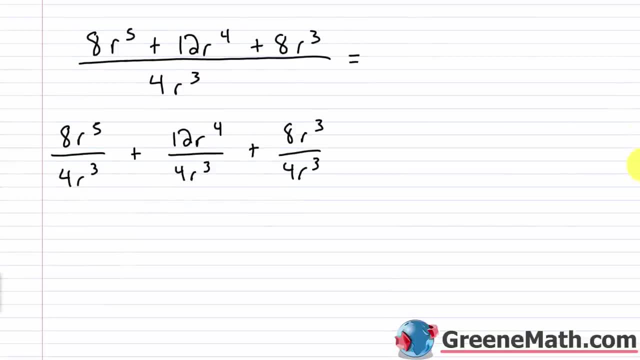 and simplify each part So let's take a look at that We know that 8r to the fifth power over 4r cubed 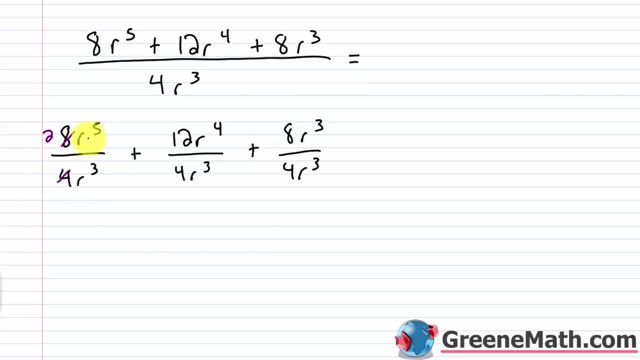 The 8 would cancel with the 4 and give me a 2 r to the fifth power over r cubed is r squared So then let's go ahead and write these as we get them So this would be 2r squared Then over here I have 12r cubed 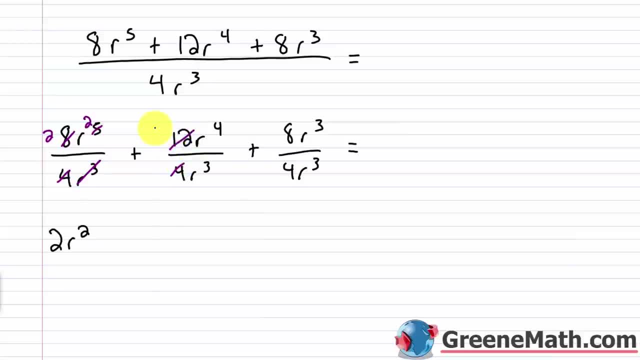 r to the fourth power over 4r cubed 12 would cancel with 4 and give me a 3 r to the fourth power over r cubed This would cancel and be r to the first power So this is plus 3r Then lastly I have 8r cubed over 4r cubed This is going to cancel with this and give me a 2 r cubed will cancel with r cubed So this will be plus 2 So I get 2r squared plus 3r plus 2 And again very very easy to check 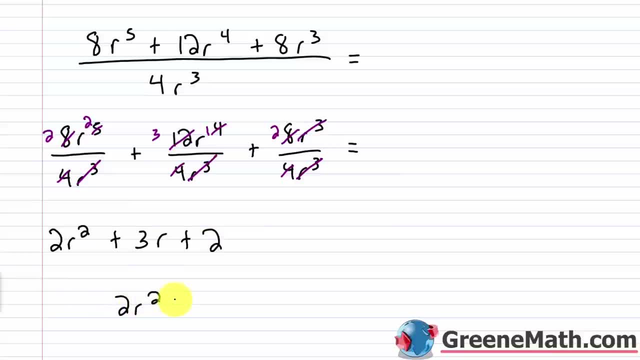 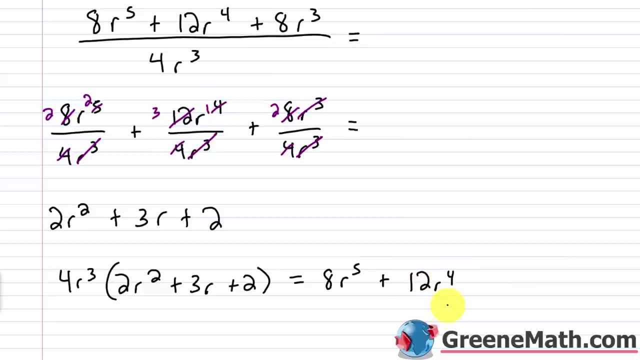 So let's take this answer here 2r squared plus 3r plus 2 This is the quotient And I want to multiply it by the divisor 4r cubed And I should get the dividend back So 4r cubed times 2r squared is 8r to the fifth power 4r cubed times 3r is plus 12r to the fourth power And then 4r cubed times 2 is plus 8r cubed 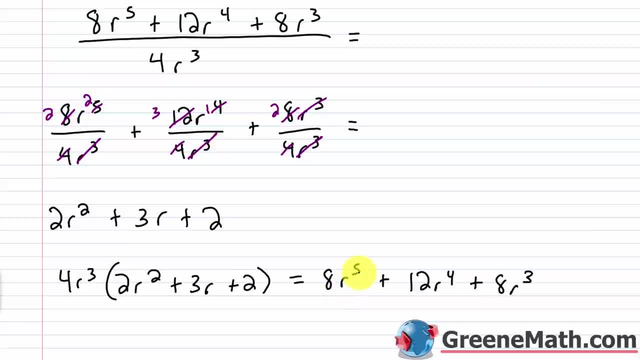 So what I get is exactly the dividend that I started with 8r to the fifth power plus 12r to the fourth power plus 8r cubed 8r to the fifth power plus 12r to the fourth power plus 8r cubed 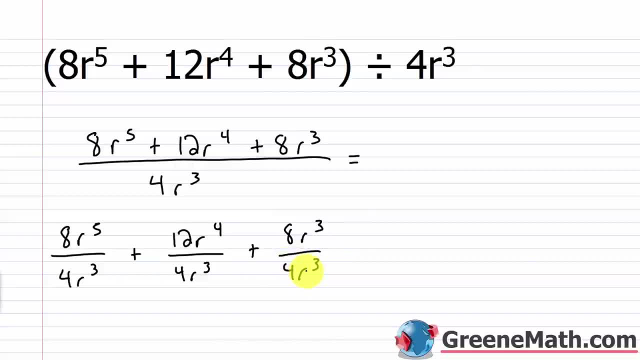 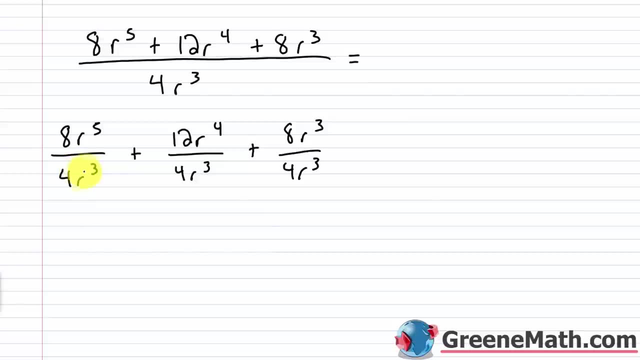 plus 8r cubed over 4r cubed. And then, once I have it in this format, it's very easy to go through and simplify each part. So let's take a look at that. We know that 8r to the 5th power over 4r cubed. the 8 would cancel out the 4 and give me a 2.. 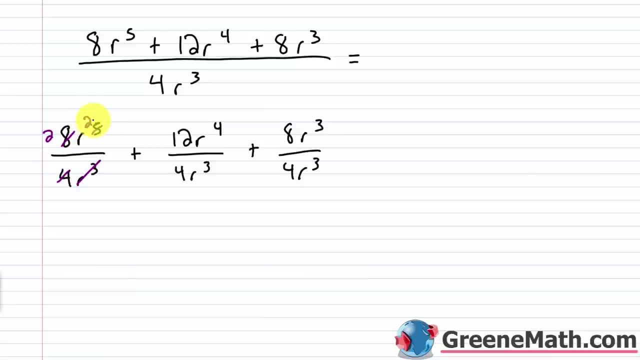 r to the 5th power over r cubed is r squared. So then let's go ahead and write these as we get them. So this would be 2r squared. Then over here I have 12r to the 4th power over 4r cubed. So I'm going to write this as 2r squared. Then over here I have 12r to the 4th power over 4r cubed. Then over here I have 12r to the 4th power over 4r cubed. 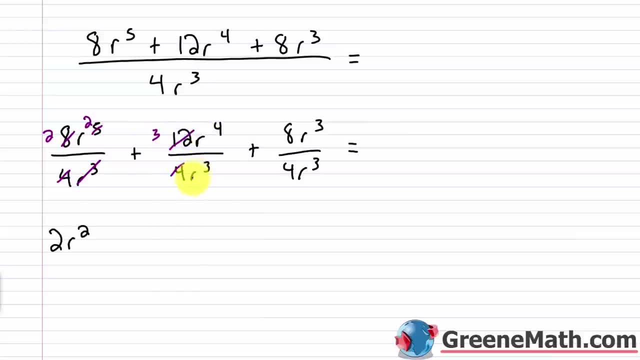 12 would cancel with 4 and give me a 3. r to the 4th power over r cubed. this would cancel and be r to the 1st power. So this is plus 3r. Then, lastly, I have 8r cubed over 4r cubed. 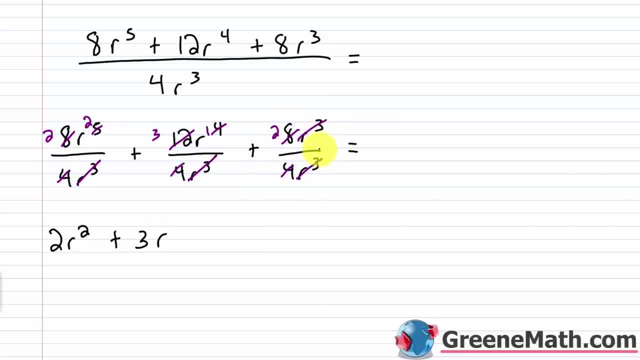 This is going to cancel with this and give me a 2. r cubed will cancel with r cubed, So this will be plus 2. So I get 2r squared plus 3r plus 2. And again, very, very easy to check. 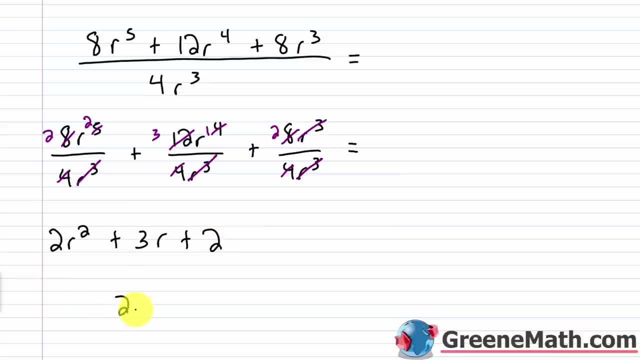 All I'm going to do is take this answer here: 2r squared plus 3r plus 2.. This is the quotient and I want to multiply it by the divisor 4r cubed and I should get the dividend back. So 4r cubed times 2r squared is 8r to the fifth power. 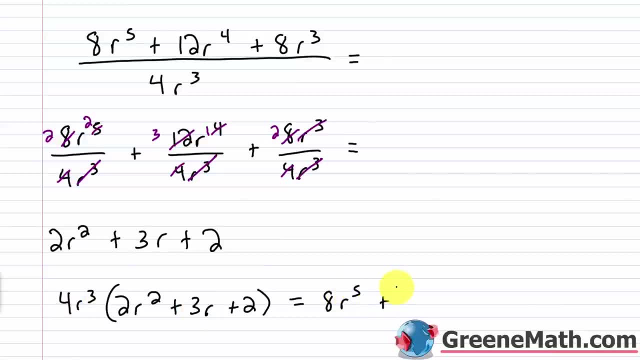 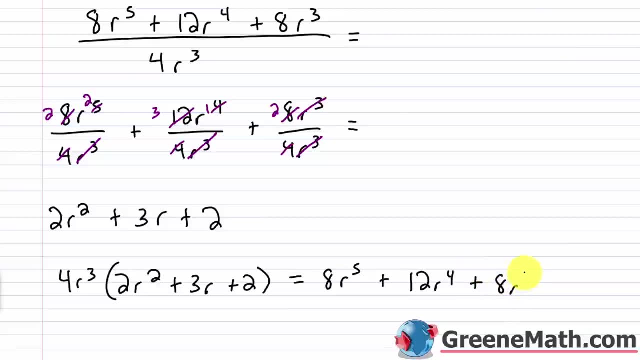 4r cubed times 3r is plus 12r to the fourth power, and then 4r cubed times 2 is plus 8r cubed. So what I get is exactly the dividend that I started with: 8r to the fifth power, plus. 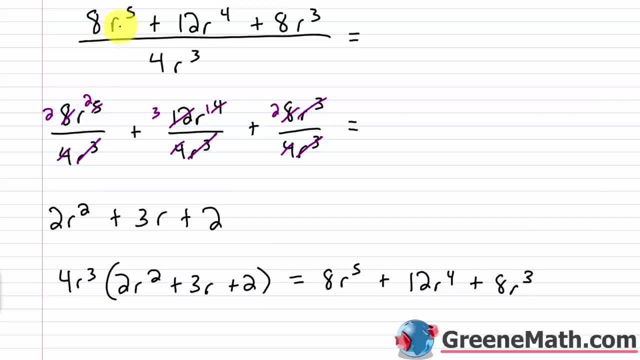 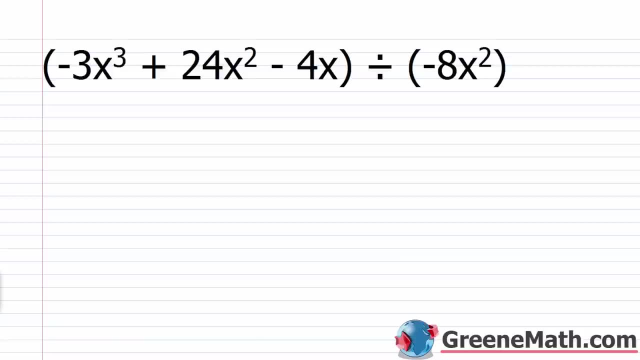 12r to the fourth power plus 8r cubed, 8r to the fifth power plus 12r to the fourth power plus 8r cubed. Let's take a look at another one. We have negative 3x cubed plus 24x squared. 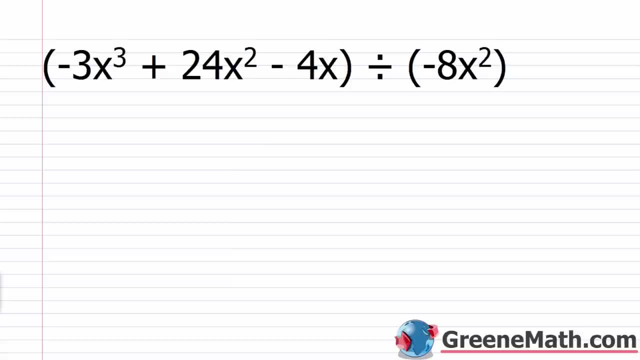 minus 4x, and then we're dividing by negative 8x squared. So I'm going to take negative 3x cubed plus 24x squared, 4x squared minus 4x. This is going to be my numerator right. That's the dividend. 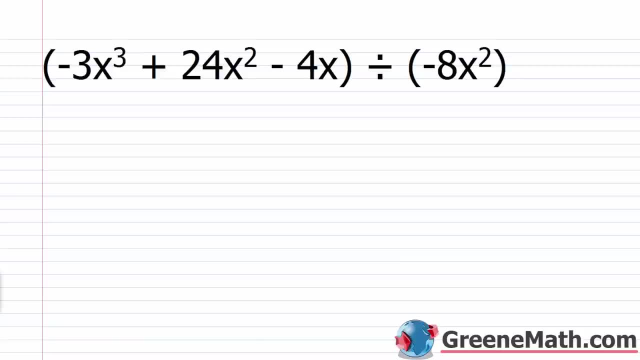 Let's take a look at another one We have negative 3x cubed plus 24x squared minus 4x And then we're dividing by 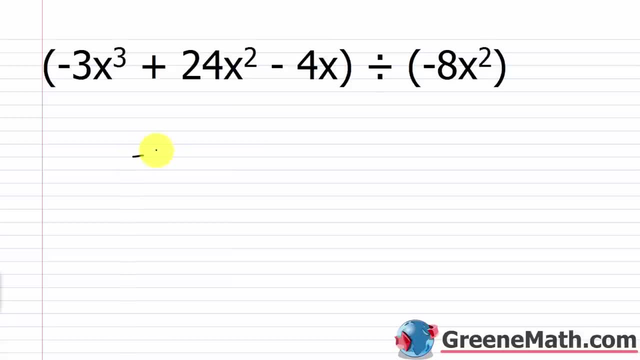 negative 8x squared So I'm going to take negative 3x cubed 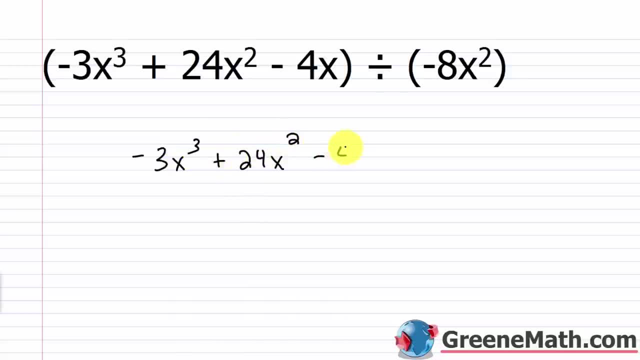 plus 24x squared minus 4x squared 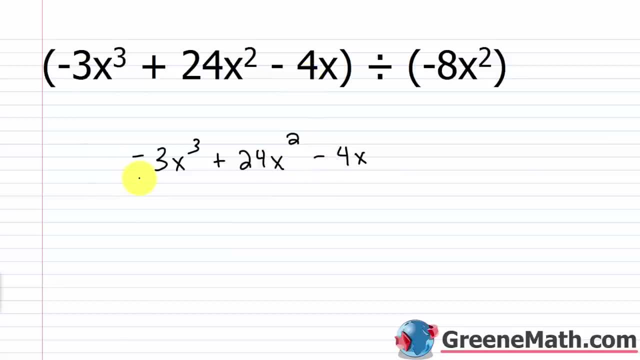 This is going to be my numerator That's the dividend And I'm dividing this by the divisor or negative 8x squared And so once I have this 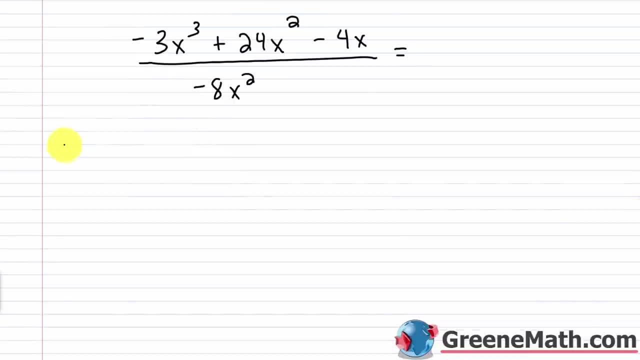 I'm just going to split it up into three different parts here So negative 3x cubed over negative 8x squared And then plus 24x squared over negative 8x squared And then I have a minus 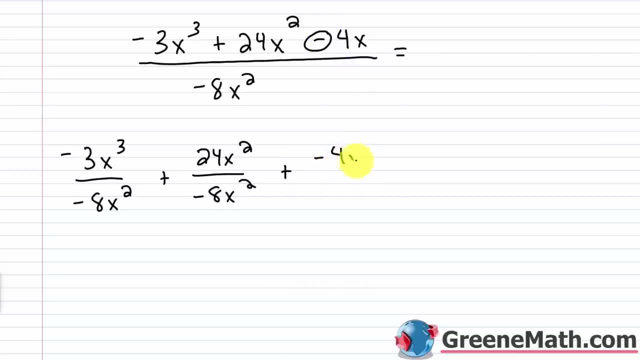 here but I think it's a little better if we put plus negative 4x over negative 8x squared 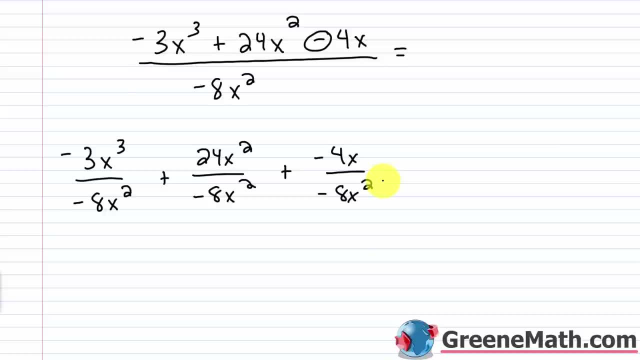 Just so we don't make a silly sign mistake 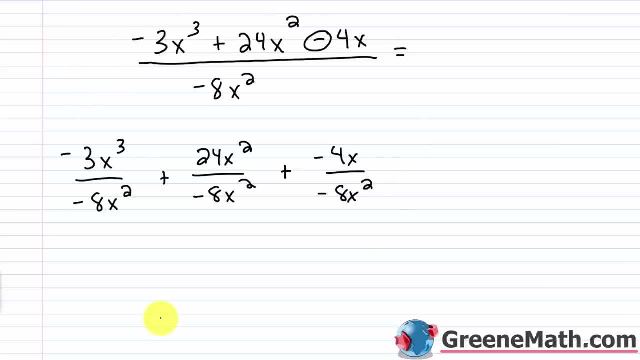 Alright, so let's take a look at this piece by piece 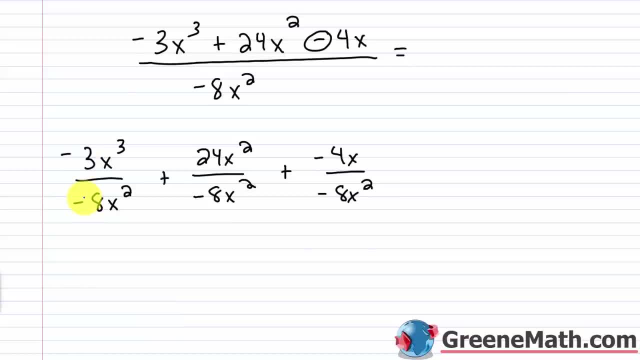 So the first thing is I have negative 3 over negative 8 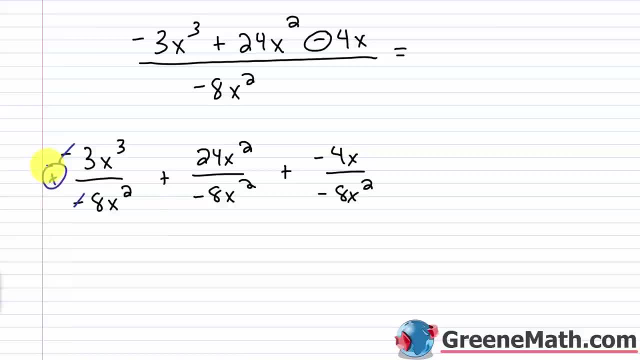 Can't really cancel anything other than the negatives Negative over negative is positive 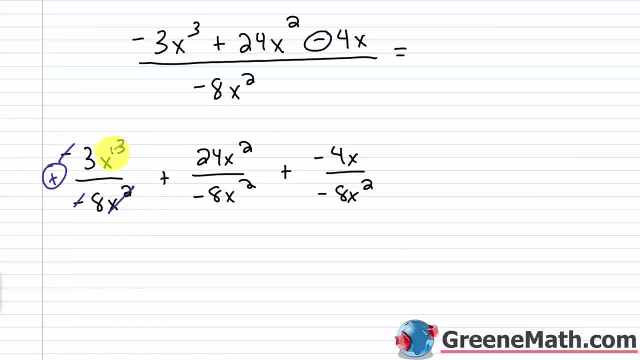 And then I have x cubed over x squared So this is going to cancel This will be x to the first power So for the first part 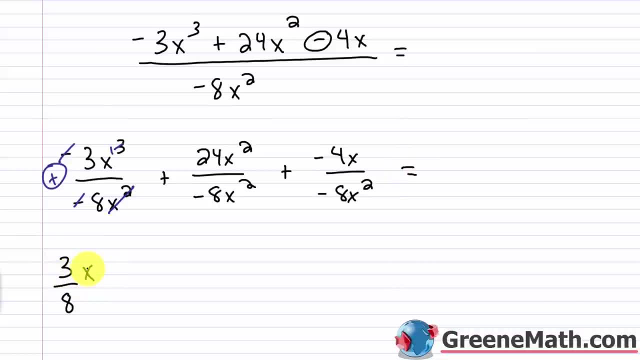 I have 3 eighths times x Or 3x over 8, you could write it that way too Doesn't really matter Then the next part we have a positive over a negative So I know that's going to be a minus 24 over 8 is 3 So this will cancel and become a 3 And we know it's negative 3 but I've already accounted for that right there 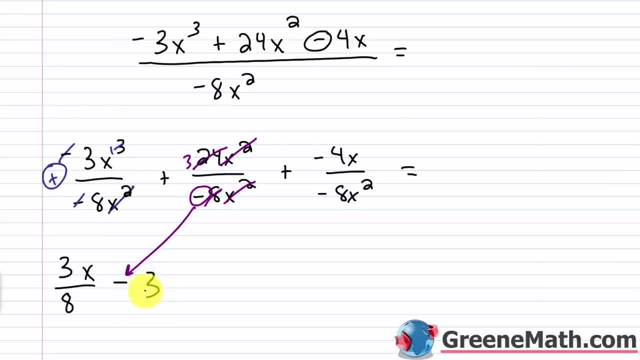 Then x squared will cancel with x squared So basically this is just minus 3 Then for the next part here 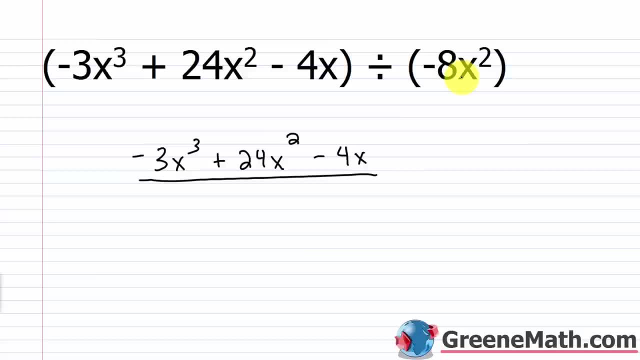 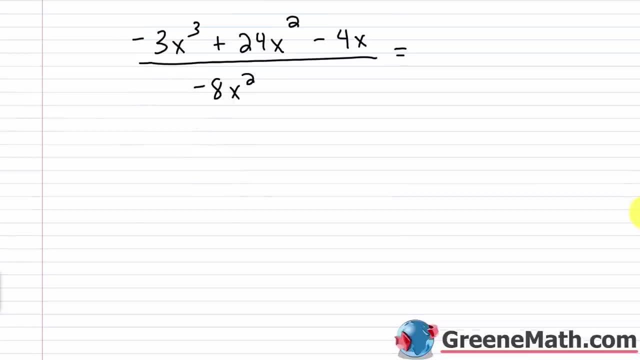 and I'm dividing this by the divisor. It's going to be my denominator: negative 8x squared, and so once I have this, I'm just going to split it up into three different parts here. So negative 3x cubed over negative 8x squared, and then plus 24x squared over negative 8x squared. 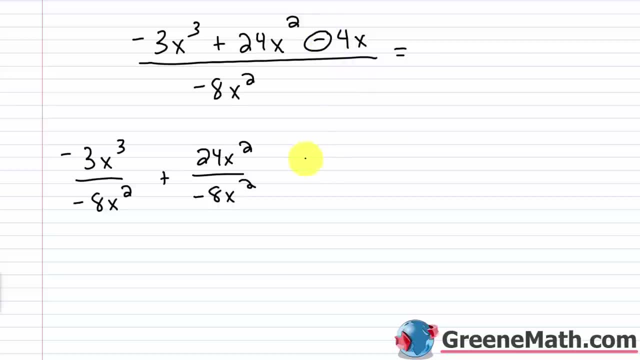 And then I have a minus here. but I think it's a little better if we put plus negative 4x over negative 8x squared, just so we don't make a silly sign mistake. All right, so let's take a look at this piece by piece. So the first thing is I have negative 3. 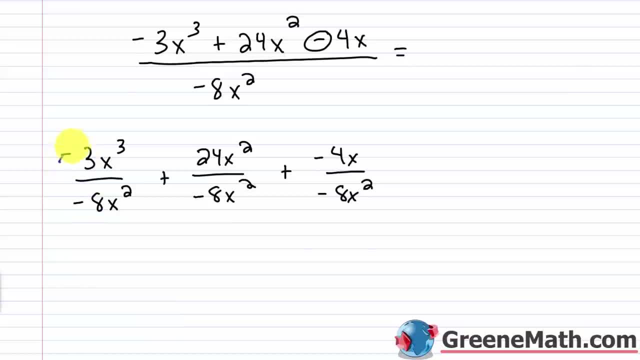 over negative 8.. Can't really cancel anything other than the negatives right, Negative over negative is positive, And then I have x cubed over x squared, So this is going to cancel This will be x to the first power. So for kind of, for the first part, we'll have 3 eighths times x, or 3x over 8.. You could write: 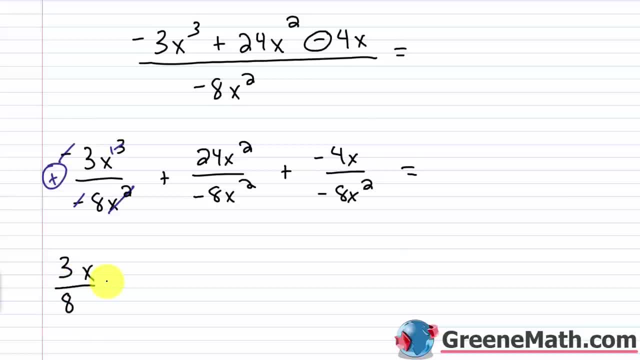 it that way too, Doesn't really matter. Then the next part. we have a positive over a negative, So I know that's going to be a minus 24 over 8 is 3.. So this will cancel, become a 3.. And 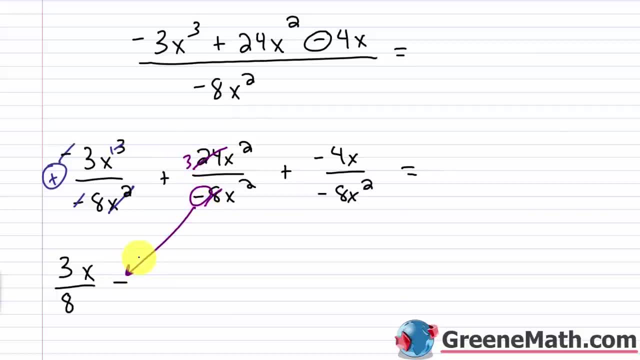 we know it's negative 3, but I've already accounted for that right there. Then x squared will cancel with x squared. So basically this is just minus 3x squared over negative x squared. Then for the next part, here I have negative 4 over negative 8.. Negative over negative is: 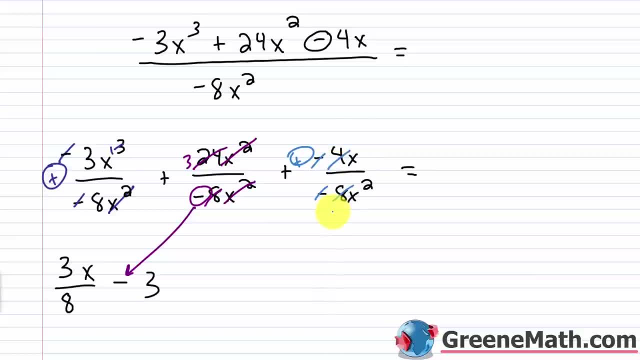 positive, And then 4 over 8.. This is going to become a 2 right here. Right because 8 divided by 4 is 2.. Now I want to look at x and x squared. This is going to cancel completely, So the. 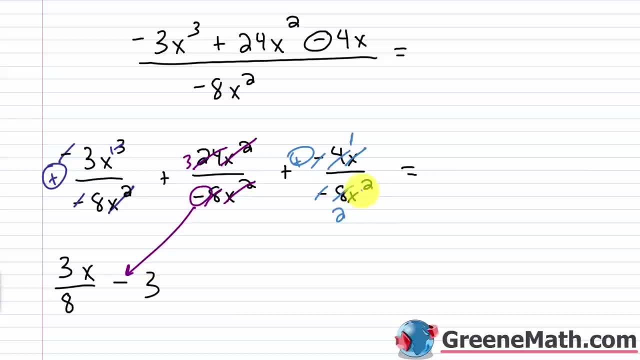 numerator is now a 1.. And then down here I'm going to take one of these factors of x away. So this would be x to the first power. So essentially what you'd have is plus 1 over 2x. And again, if we want to check this, we'll take this quotient here and multiply. 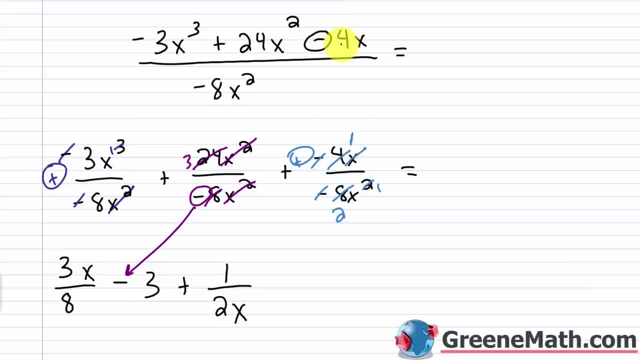 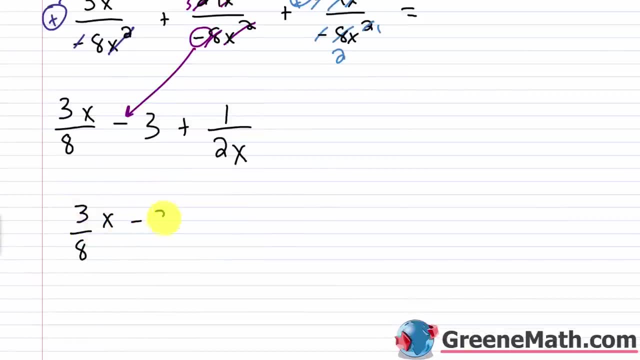 it by the divisor And it should give me this dividend back. So let's try that real quick. So we'll do 3 eighths x minus 3 plus 1 over 2x, And we're multiplying this by the divisor. 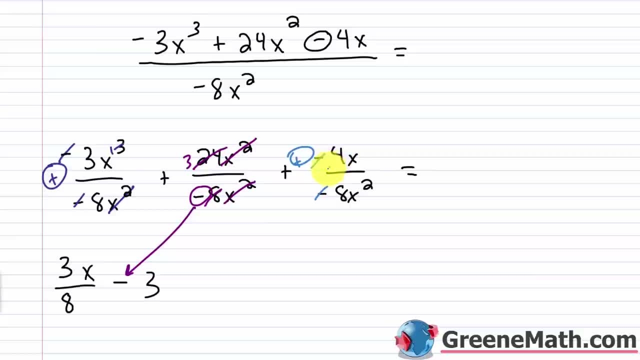 I have 4 over negative 8 Negative over negative is positive And then 4 over 8 This is going to become a 2 right here Because 8 divided by 4 is 2 Now when I look at x and x squared This is going to cancel completely So the numerator is now a 1 And then down here I'm going to take one of these factors of x away, so this would be x to the first power So essentially what you'd have is plus 1 over 2x And again 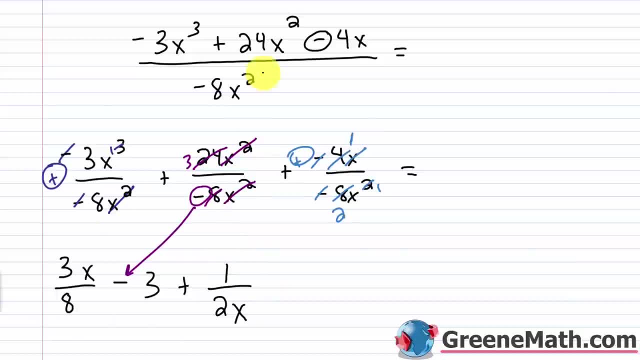 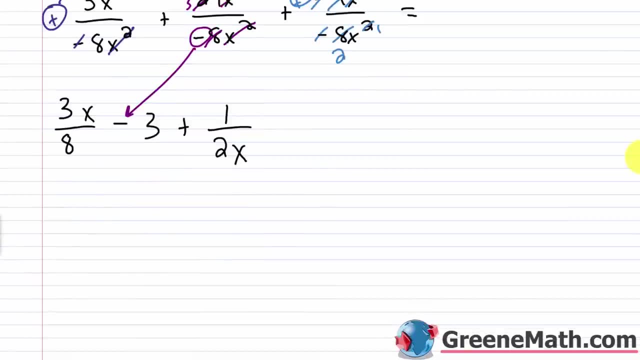 If we want to check this We'll take this quotient here And multiply it by the divisor And it should give me this dividend back So let's try that out real quick So we'll do 3 eighths x minus 3 plus 1 over 2x And we're multiplying this by the divisor which was negative 8x squared So let's see what this gives us So negative 8x squared times 3 eighths x 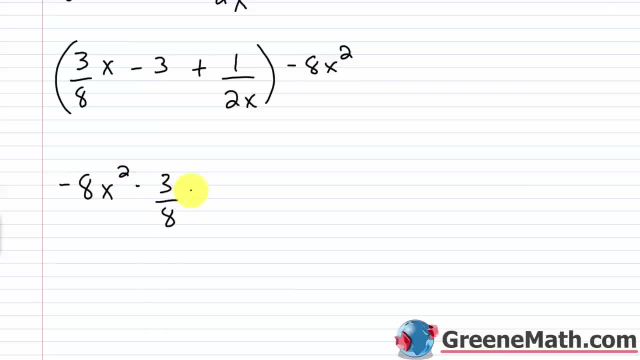 Let me write that out so you can see what's going to cancel So obviously this 8 will cancel with this 8 I'll basically just have a negative 1 there Negative 1 times 3 is negative 3 So that's negative 3 And then x squared times x is x cubed Then next I have negative 3 times negative 8x squared Negative times negative is positive 3 times 8 is 24 So plus 24x squared Then lastly I have 8x squared times 1 over 2x So negative 8x squared 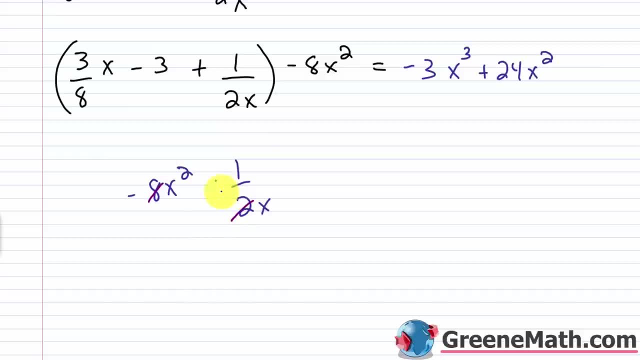 Times 1 over 2x This is going to cancel with this And give me a 4 And x squared over x This would cancel with one of these So basically I'd have negative 4x there So minus 4x And we can scroll back up And see that that is our dividend Negative 3x cubed plus 24x squared Minus 4x Alright let's take a look at another one 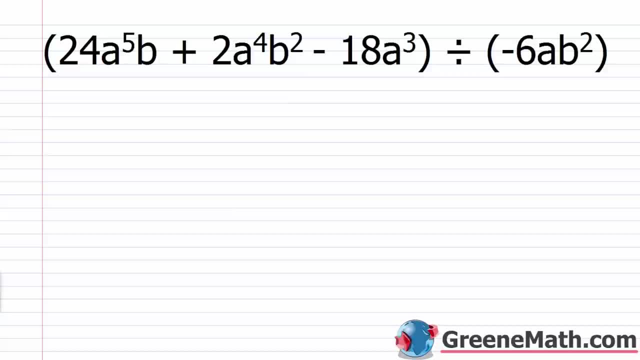 24a to the 5th power b Plus 2a to the 4th power b squared Minus 18a cubed 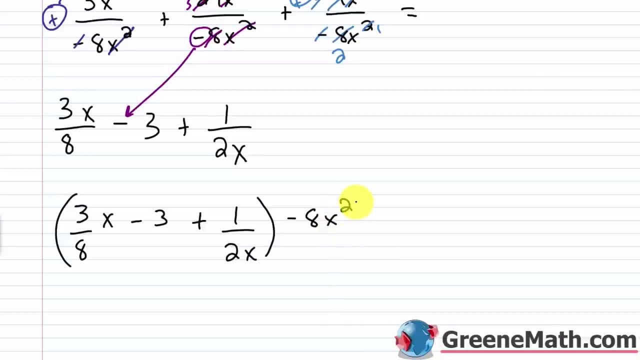 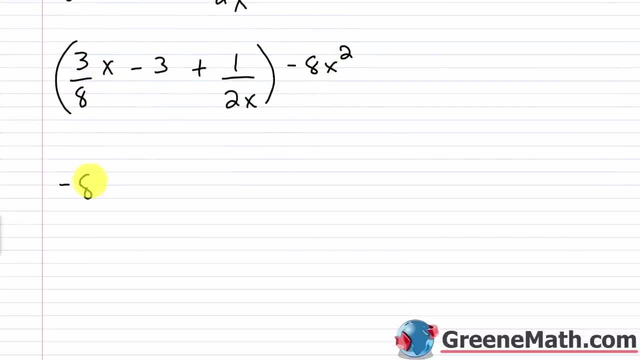 which was negative 8x squared. So let's see what this gives us. So negative 8x squared times 3 eighths x. So let me write that out so you can see what's going to cancel. So obviously this 8 will cancel with this 8.. I'll basically just have a negative 1 there. 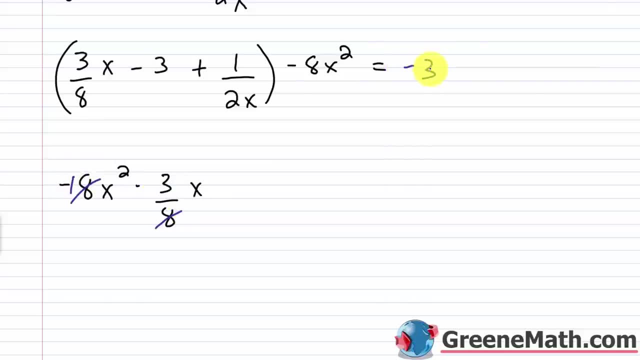 Negative 1 times 3 is negative 3.. So that's negative 3.. And then x squared times x is x cubed. Then next I have negative 3 times negative. 8x squared. Negative times negative is positive 3 times 8 is 24.. So plus 24x squared. 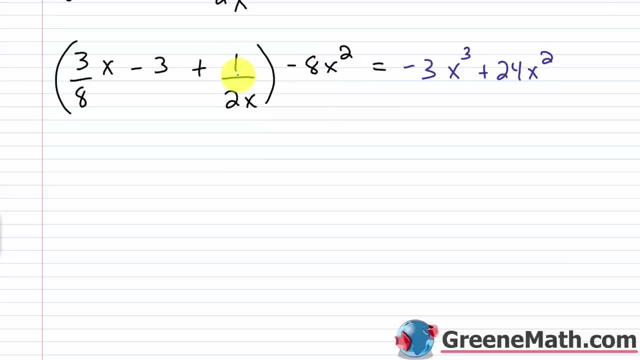 Then, lastly, I have negative 8x squared times 1 over 2x. So negative 8x squared times 1 over 2x. This is going to cancel with this and give me a 4.. And x squared over x. this would cancel with. 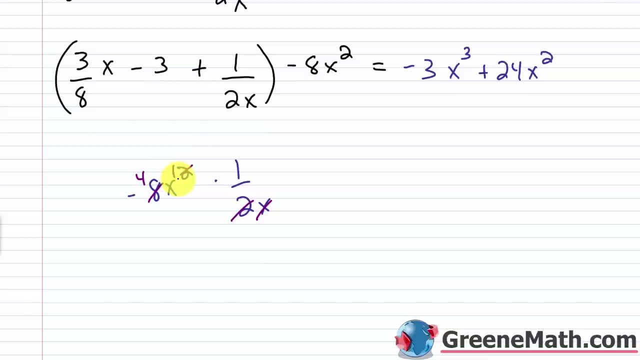 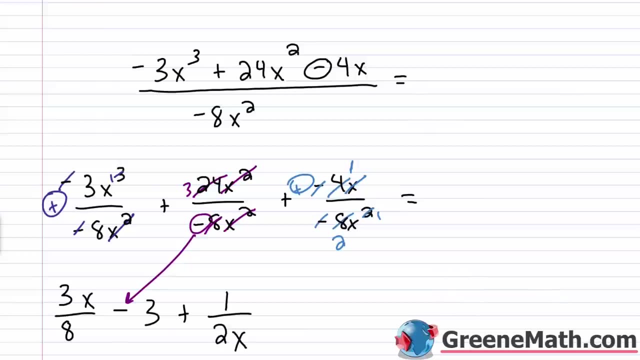 one of these. So basically I'd have negative 4x there, So minus 4x, And we could scroll back up and see that that is our dividend: Negative 3x cubed plus 24x squared, minus 4x. All right, let's. 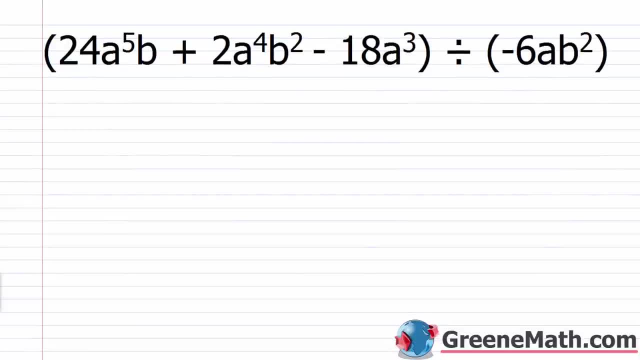 take a look at another one. We can see that this is our dividend. So we can see that this is our dividend. We have 24a to the 5th power b plus 2a to the 4th power b, squared, minus 18a cubed, And then this is: 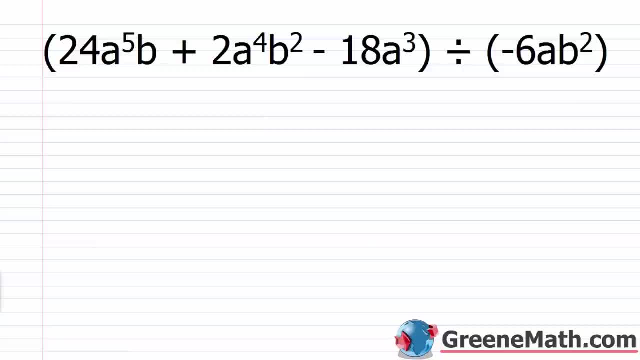 divided by negative 6ab squared. So let's kind of shortcut this And instead of writing this as a fraction and then kind of splitting it up, let's just split it up right away. So I'm going to take this term right here, This 24a to the 5th power b, And write it over the divisor here: Negative. 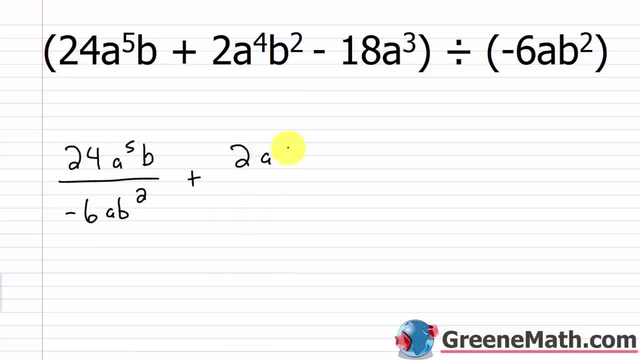 6ab squared, Then plus, I'm going to have 2a to the 4th power b squared over that divisor. Negative, 6ab squared. And then I have that minus- Let me put plus negative- 18a cubed over again negative. 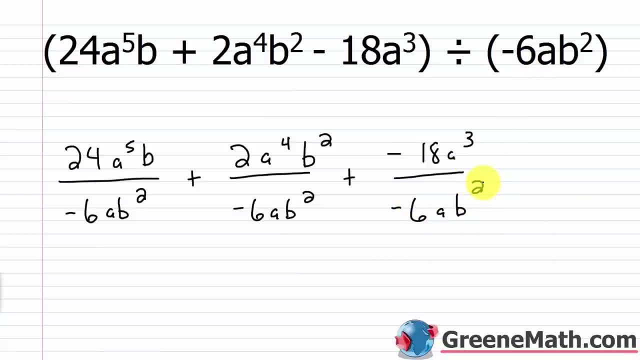 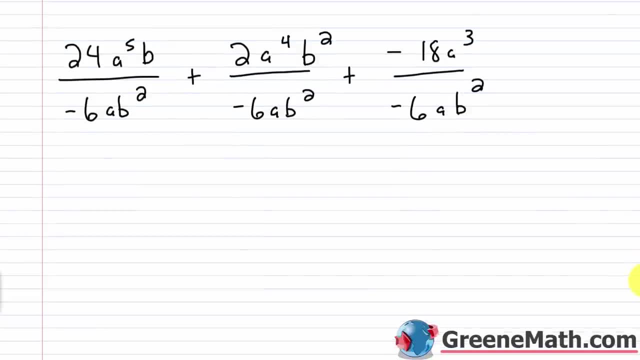 6ab squared, Anything I can do to kind of give you a shortcut, Because a lot of times you're going to be doing this on a timed exam And you don't want to take two steps when you can do something in one time. So I'm going to take 2a to the 4th power b squared And then I'm going to 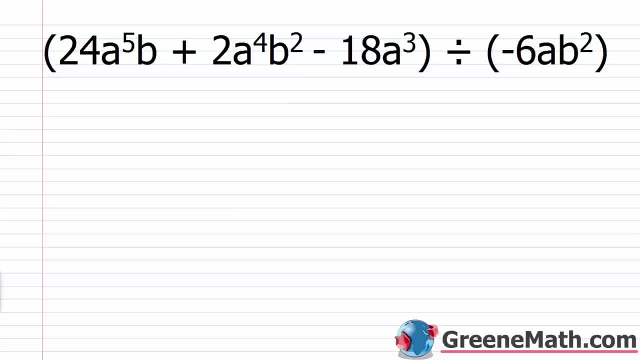 And then this is divided by Negative 6ab squared So let's kind of Shortcut this And instead of writing this as a fraction And then kind of splitting it up Let's just split it up right away So I'm going to take this term right here This 24a to the 5th power b And write it over The divisor here Negative 6ab squared Then plus I'm going to have 2a to the 4th power b squared Over 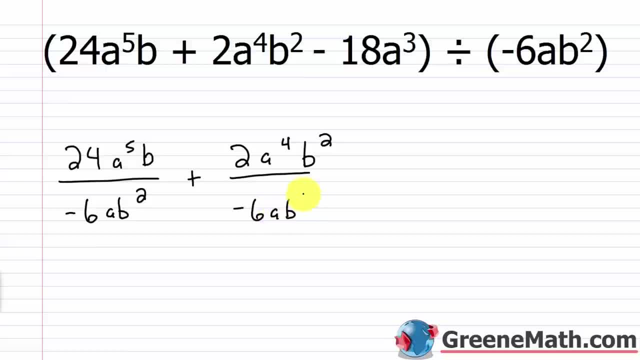 That divisor Negative 6ab squared And then I have that minus 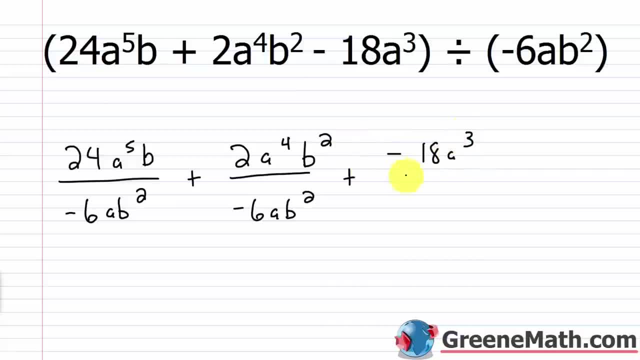 Let me put plus negative 18a cubed 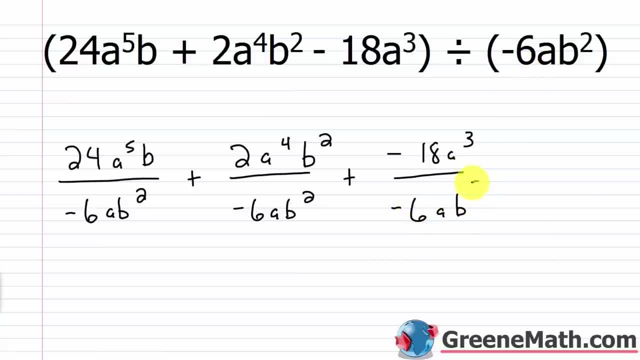 Over Again negative 6ab squared 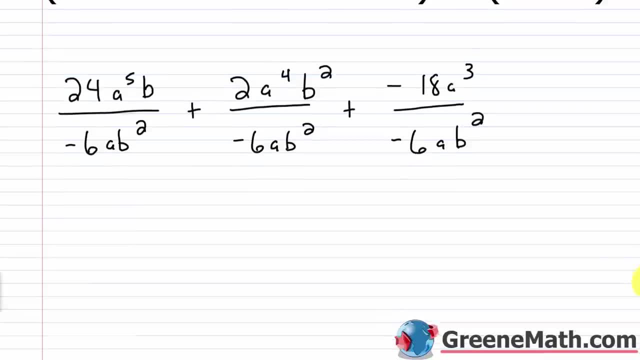 Anything I can do to kind of give you a shortcut Because a lot of times You're going to be doing this on a timed exam And you don't want to take two steps When you can do something in one 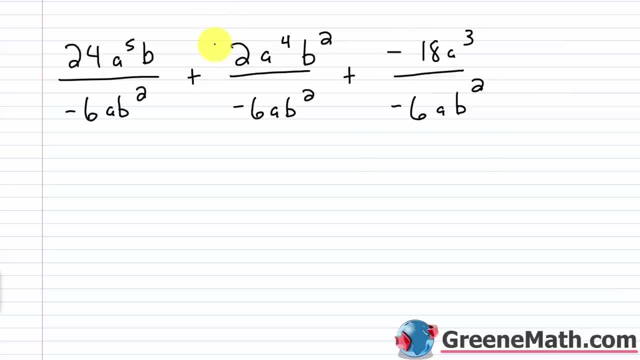 So let's simplify each part Kind of separately 24 over negative 6 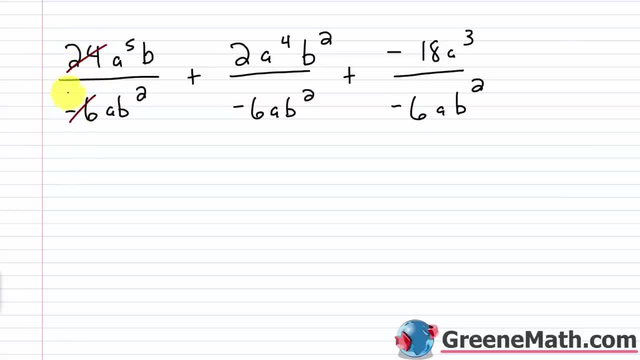 Would be negative 4 So this would cancel with this And it would be negative 4 Then a to the 5th power over a This would cancel and this would be a to the 4th power Then b over b squared This would cancel and this would be b to the 1st power So kind of the first part here Would be negative 4 a to the 4th power Over b Then if I move on over here 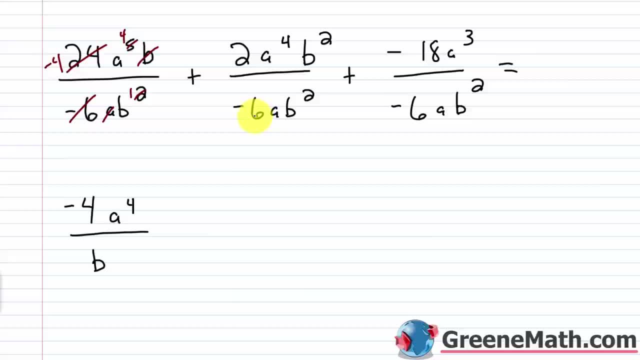 I see that I have 2 over negative 6 I know this is going to be negative So let me just go ahead and put a negative out in front 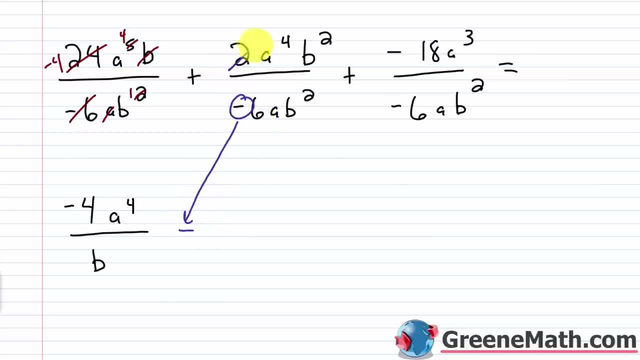 That's going to go right there 2 over 6 This is going to be a 1 And this is going to be a 3 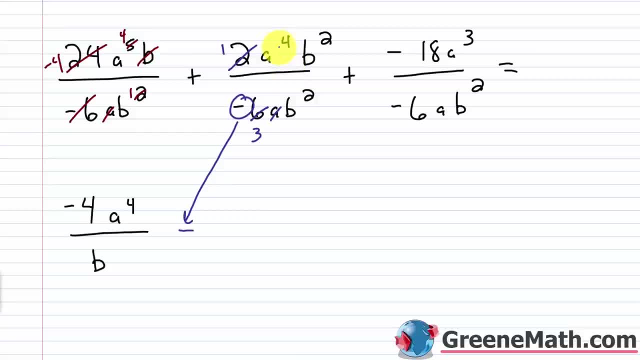 6 divided by 2 is 3 Then we have a to the 4th power over a 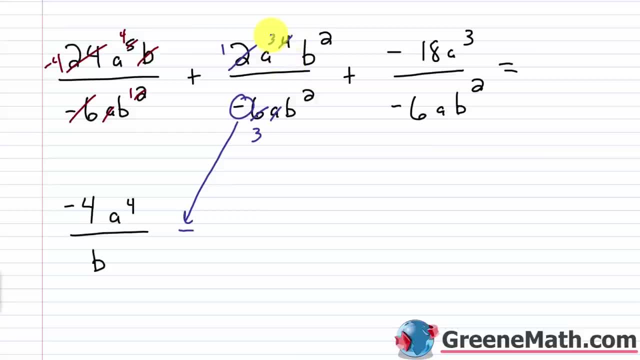 This is going to cancel with one of these So instead of 4 this will be 3 And then b squared will cancel with b squared So what I'll have here I have the minus 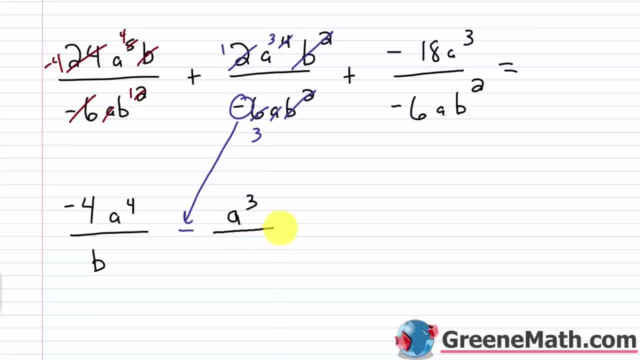 Then I'll have a cubed In the numerator over In the denominator I'll just have a 3 Right I've already accounted for that negative 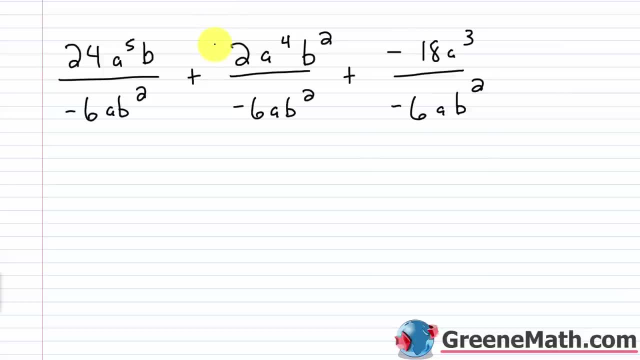 write it over the divisor here: Negative 1.. So let's simplify each part kind of separately: 24 over negative 6 would be negative 4.. So this would cancel with this And it'd be negative 4.. Then a to the 5th power over a. This would cancel And this would be a to the 4th power. Then b over b. 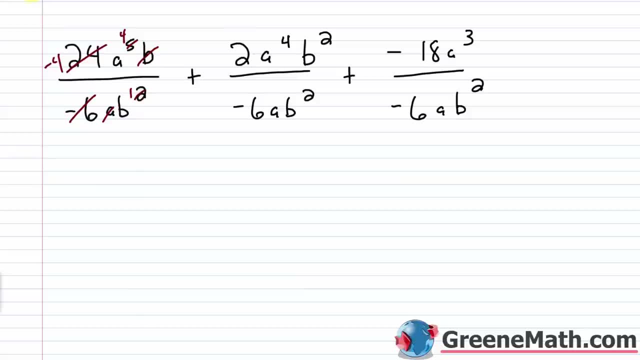 squared. This would cancel And this would be b to the 1st power. So kind of the first part here would be negative 4: a to the 4th power over b. Then if I move on over here I see that I have 2 over negative 6.. I know this is going to be. 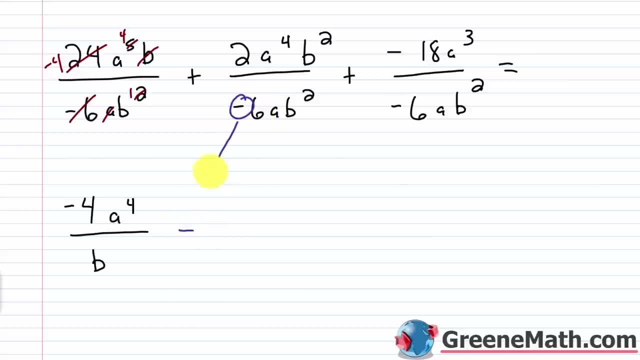 negative. So let me just go ahead and put a negative out in front. That's going to go right there. 2 over 6.. This is going to be a 1.. And this is going to be a 3.. 6 divided by 2 is 3.. 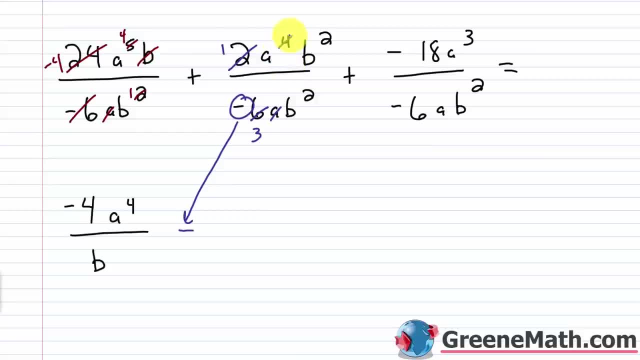 Then we have a to the 4th power over a. This is going to cancel with one of these. So instead of 4, this will be 3.. And then b squared will cancel with b squared. So what I'll have here? I have the. 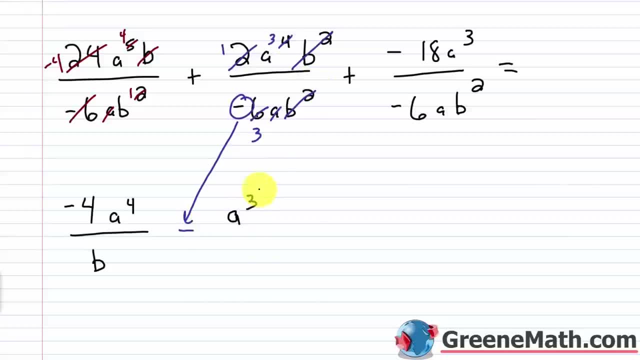 minus, And then I'll have a cubed In the numerator over In the denominator. I'll just have a 3.. I've already accounted for that negative, All right, Then next I move on over here. I have a negative over a negative, I know. 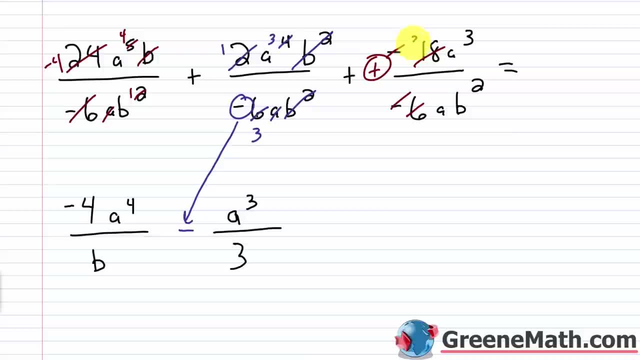 that's going to be positive. And then 18 over 6 is 3.. a cubed over a. This is going to be a squared And then b squared. I don't have anything to kind of match up with that, So that's just going to. 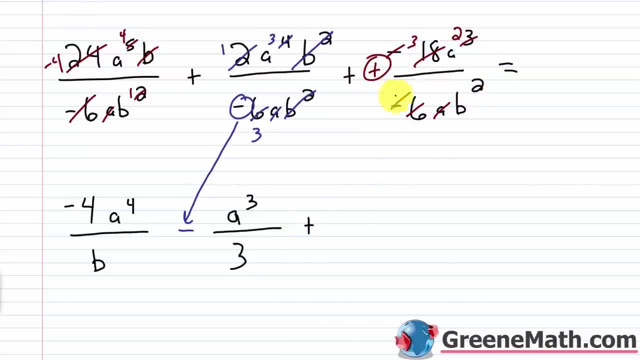 stay All right. So then it's going to be plus. We have 3. a squared over in the denominator, b squared. So here's our answer: Negative 4a to the 4th power over b, minus a cubed over 3, plus 3a squared over b squared. So I'm not going to check this one, just 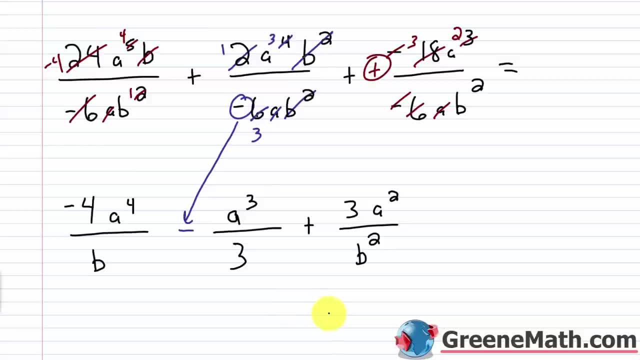 in the interest of time, But go ahead and pause the video. if you're interested, Take your quotient here. The negative 4a to the 4th power over b minus a cubed over 3 plus 3a squared over b squared. 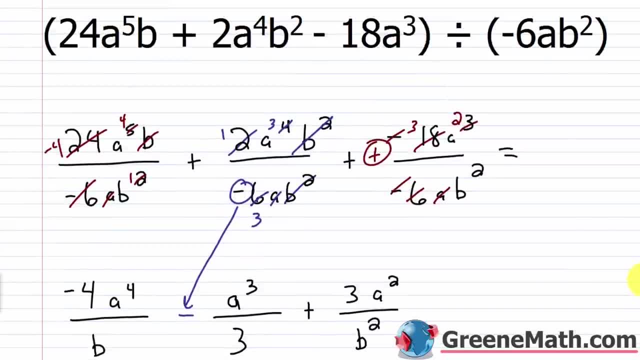 Multiply it by the divisor. Okay, Multiply. Multiply it by the divisor, which we know is negative, 6ab squared, And you will get the dividend back: 24a to the 5th power b, plus 2a to the 4th power b squared, minus 18a cubed, So go. 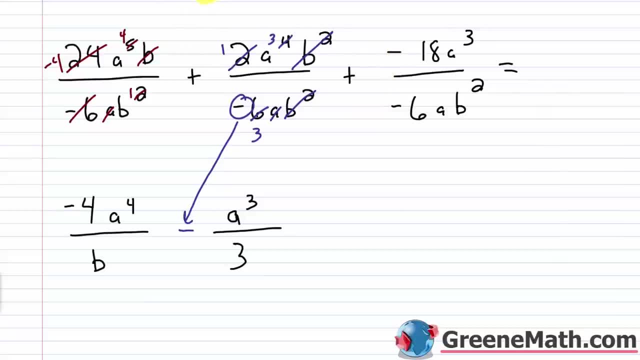 Alright then next I move on over here I have a negative over a negative I know that's going to be positive And then 18 over 6 is 3 a cubed over a This is going to be a squared And then b squared I don't have anything to Kind of match up with that so that's just going to stay Alright so then It's going to be plus Then I have 3 a squared over In the denominator b squared So here's our answer 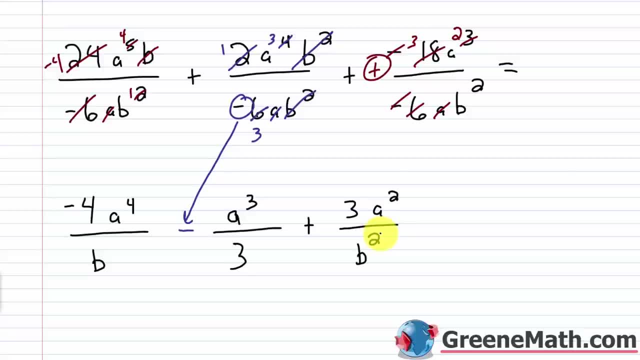 Negative 4 a to the 4th power over b Minus a cubed over 3 Plus 3 a squared over b squared 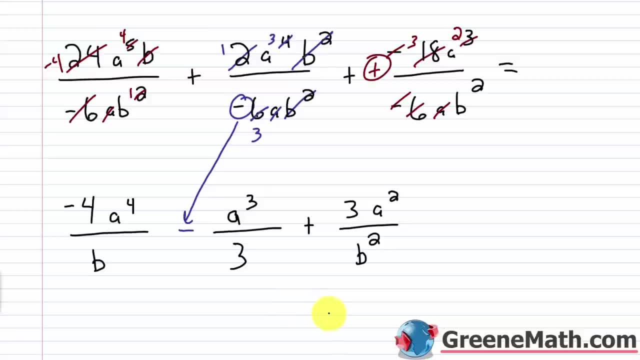 So I'm not going to check this one just in the interest of time But go ahead and pause the video if you're interested 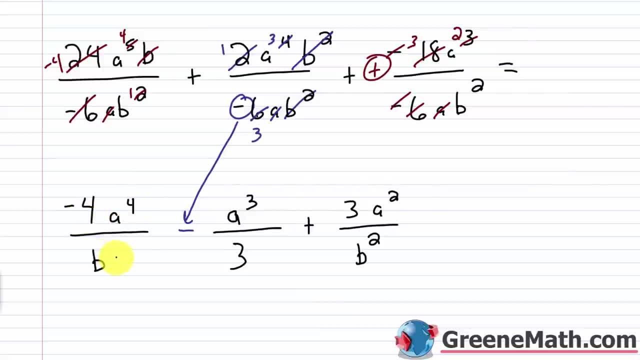 Take your quotient here The negative 4 a to the 4th power over b 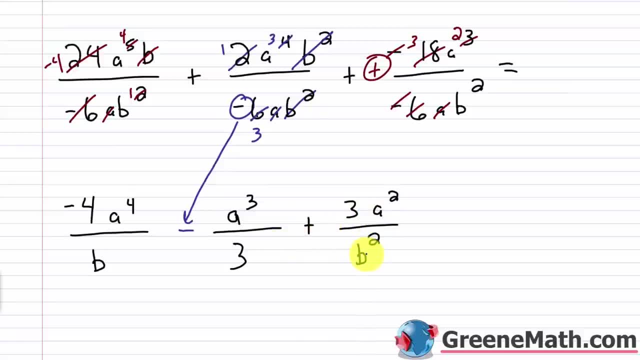 Minus a cubed over 3 Plus 3 a squared over b squared 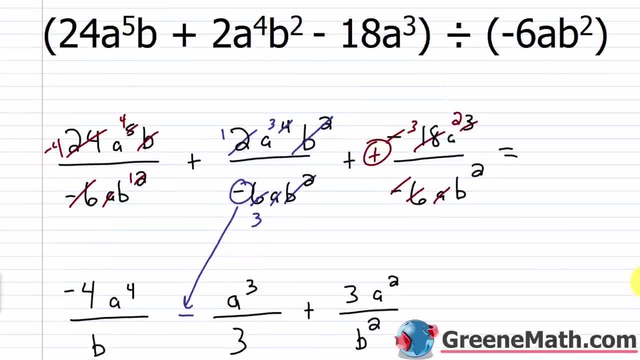 Multiply it by the divided Okay multiply it by the divisor Which we know is negative 6 a b squared 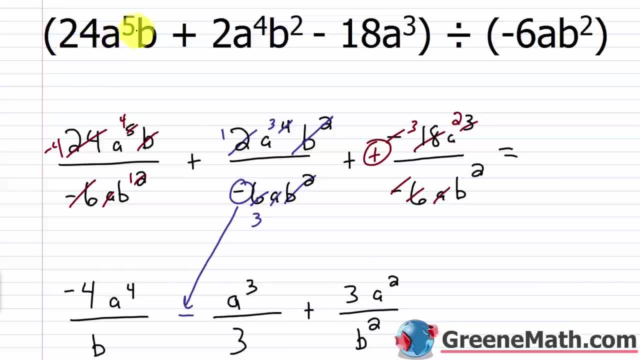 And you will get the dividend back 24 a to the 5th power over b 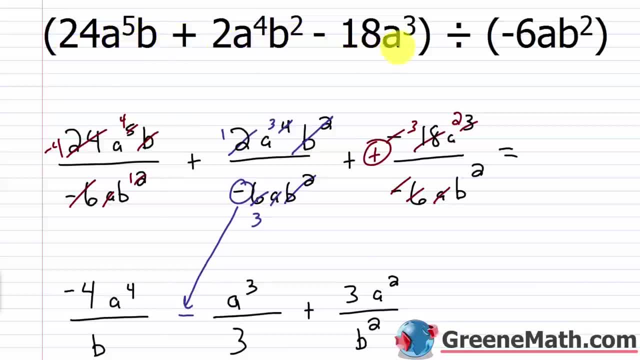 Plus 2 a to the 4th power over b squared Minus 18 a cubed So go ahead and pause the video if you want 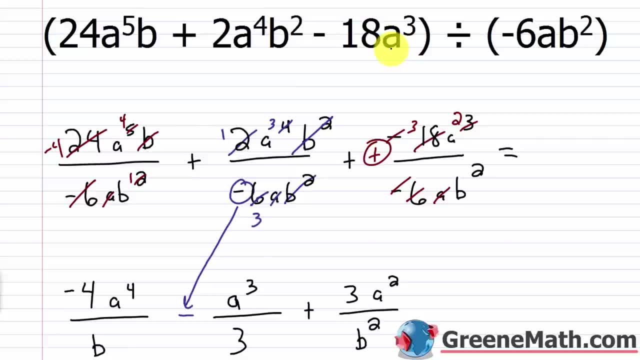 Take a look at that And then we're going to do one more problem 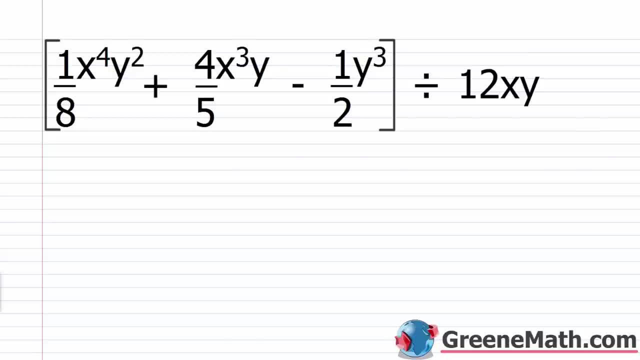 Alright for the last one I have 1 eighth x to the 4th power over y squared 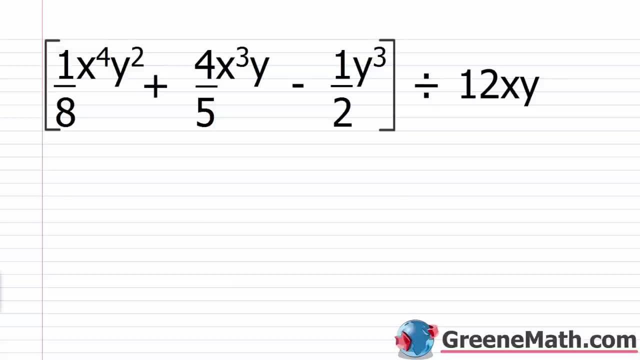 Plus 4 fifths x cubed y Minus 1 half y cubed This is divided by 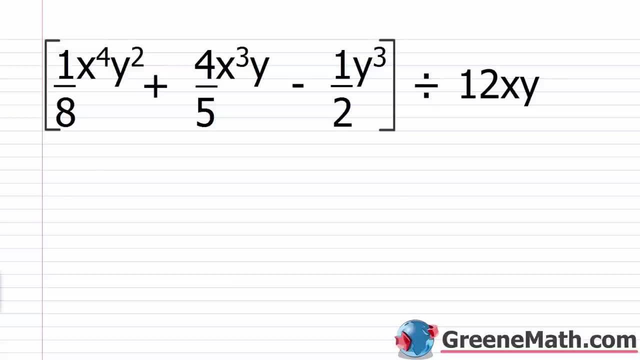 12 x y Now before we kind of look at this 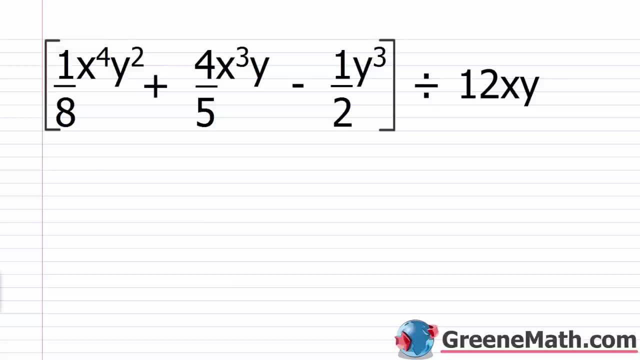 I want you to recall that If you're dividing a fraction 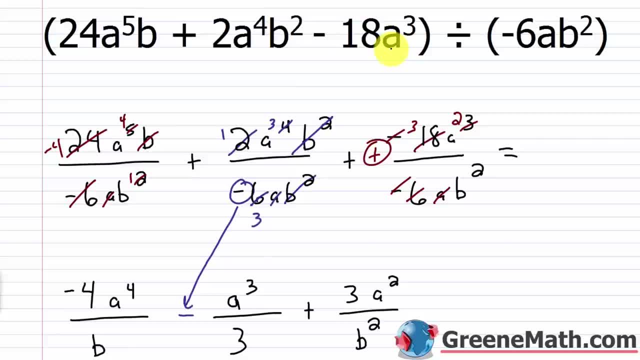 ahead and pause the video. if you want, Take a look at that, And then we're going to do one more problem. All right, For the last one, I have 1 eighth x to the 4th power, y squared plus 4 fifths. 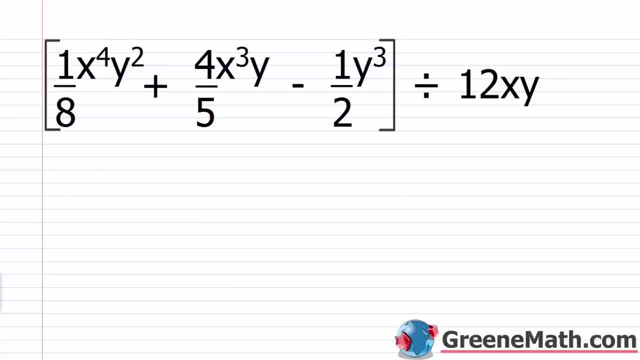 x cubed, y minus 1 half y cubed, And this is divided by 12xy. Now, before we come back to look at this, I want you to recall that if you're dividing a fraction, so something like 3 fourths- 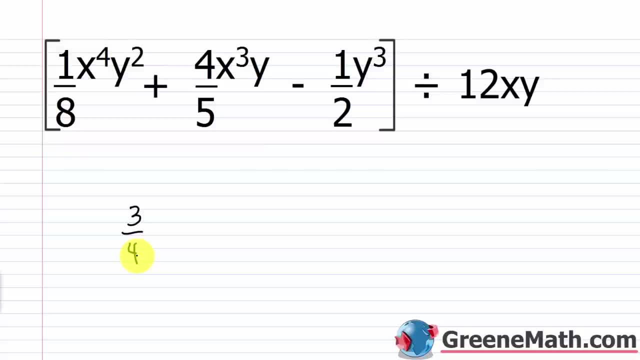 by a number or another fraction. how do we do it? We take the first fraction, We multiply by the reciprocal of the second. So if I had 3 fourths divided by, let's say, 10, I would say this is 3 fourths times the reciprocal of 10, which is 1 tenth. And you could write this as: 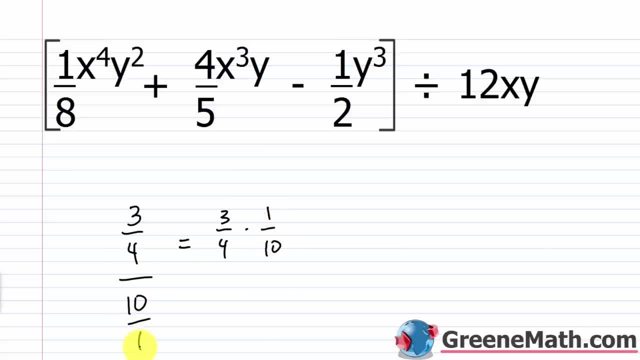 10 over 1, if that makes it easier for you. So instead of sitting here and saying, okay, I have 1 x to the 4th power, y squared over 8. And this is divided by 12xy. I know in the end. 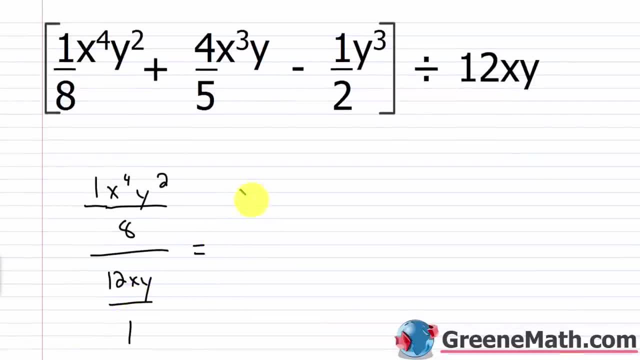 I'm going to write this over 1.. And this is going to be equal to x, to the 4th power, y, squared over 8 times the reciprocal of this guy, which is 1 over 12xy. I can just start out. I can make this. 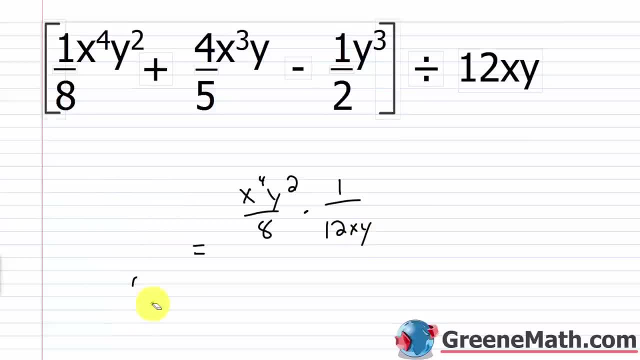 much simpler and write this as kind of a multiplication problem. I can see this and say, well, instead of dividing by 12xy, I can kind of say this is times 1 over 12xy. It's the same thing If I were to multiply 20 by 1 half. 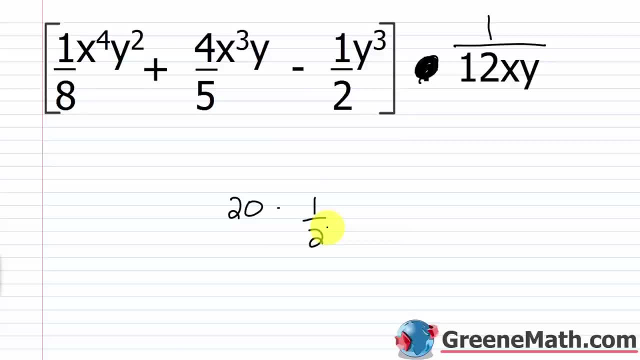 it's the same thing as if I divided 20 by 2, right Same thing. So doing it this way is just going to make it simpler for us. We would have x to the 4th power, y squared over 8 times. 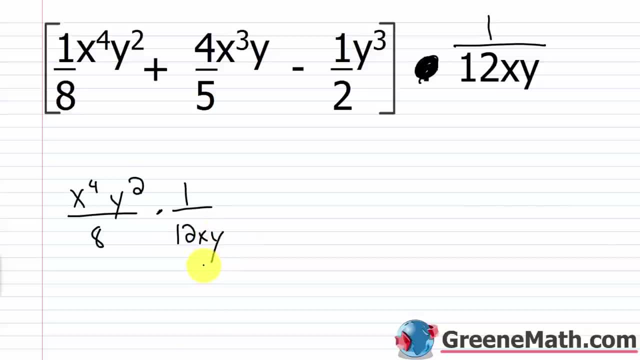 times 1 over 12xy. Again, if I did it using division, after I do my, multiply the first guy by the reciprocal of the second, I end up with this anyway. So I might as well start out doing that Again. if you have something that normally takes two steps, if you can cut it down to one. So something like 3 fourths 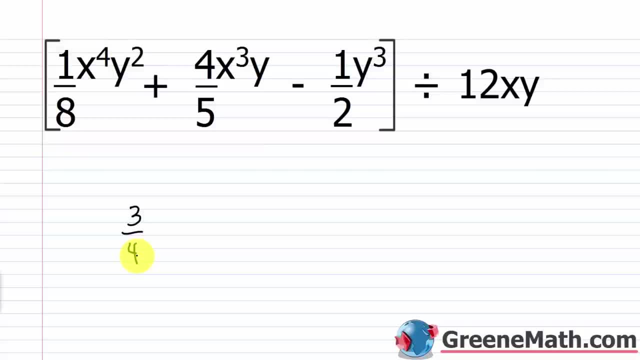 By a number or another fraction How do we do it We take the first fraction We multiply by the reciprocal of the second So if I had 3 fourths divided by Let's say 10 I would say this is 3 fourths times The reciprocal of 10 which is 1 tenth 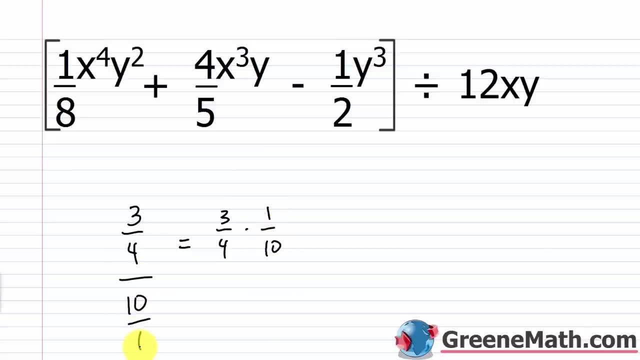 And you could write this as 10 over 1 If that makes it easier for you 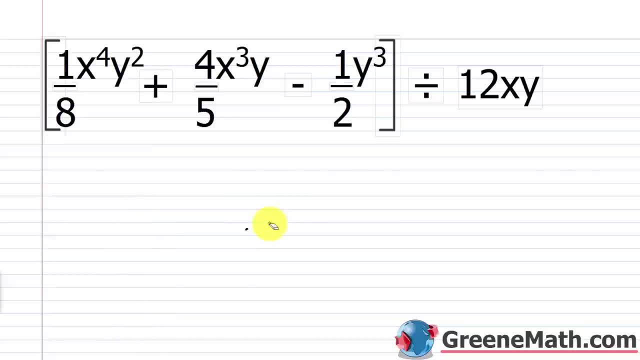 So instead of sitting here And saying okay I have 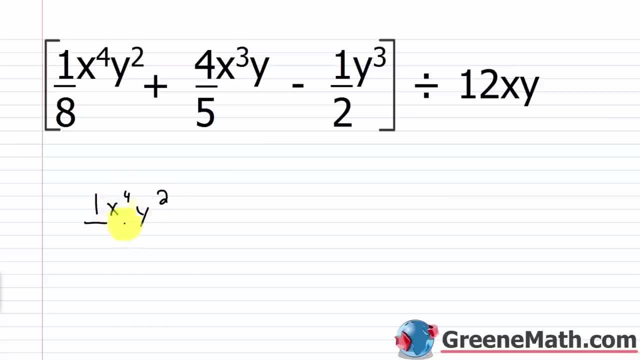 1 x to the 4th power Y squared 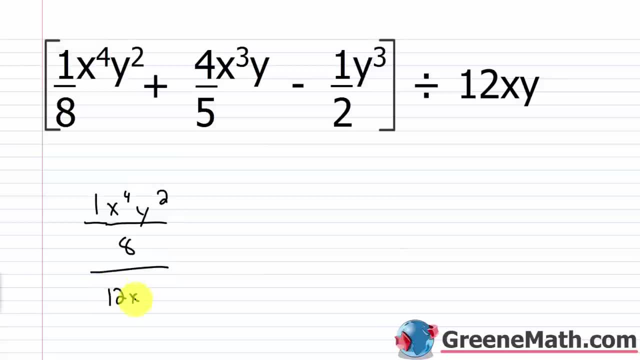 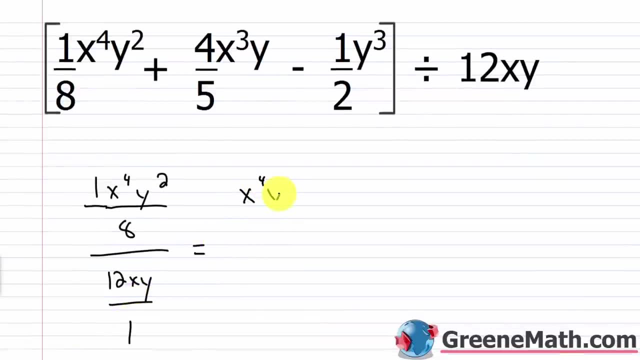 Over 8 And this is divided by 12 x y I know in the end I'm going to write this over 1 And this is going to be equal to x to the 4th power y squared over 8 Times the reciprocal of this guy Which is 1 over 12 x y I can just start out I can make this much simpler And write this as kind of a multiplication problem I can see this And say well instead of Dividing by 12 x y I can kind of 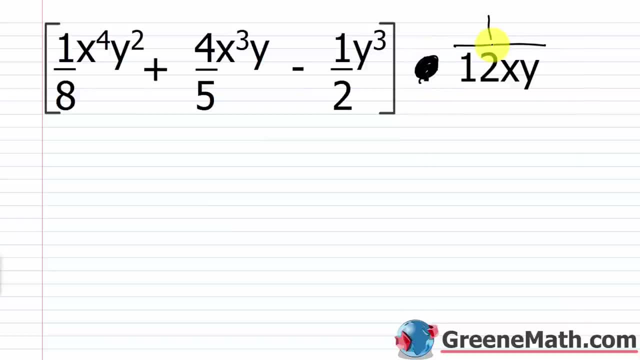 Say this is times 1 over 12 x y It's the same thing If I were to multiply 20 By 1 half It's the same thing as if I divided 20 by 2 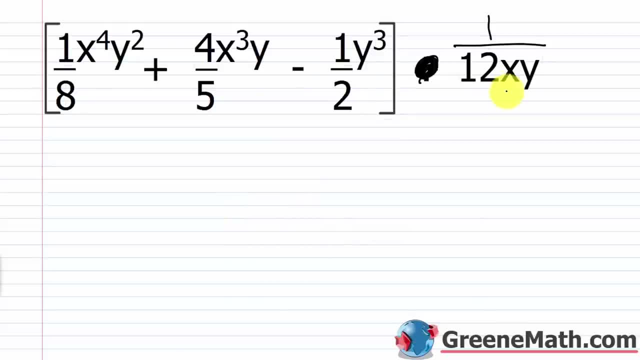 Same thing So doing it this way 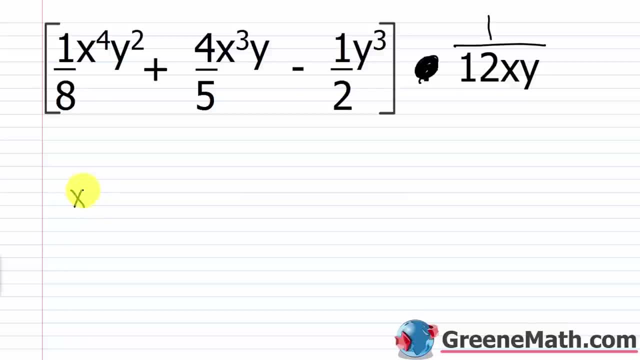 Is just going to make it simpler for us We would have x to the 4th power y squared over 8 Times 1 over 12 x y 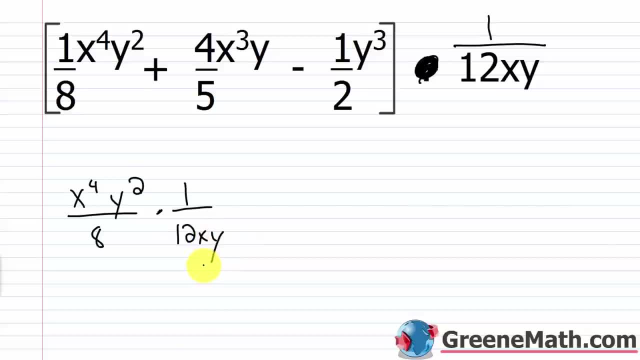 Again if I did it using division After I do my Multiply the first guy 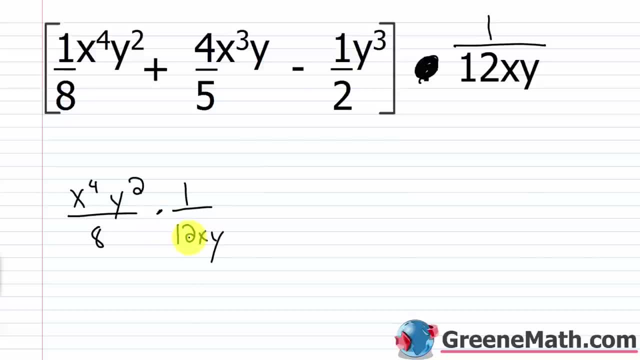 By the reciprocal of the second I end up with this anyway So I might as well start out doing that Again if you have something that normally takes 2 steps If you can cut it down to 1 It's just going to put you one step ahead Alright then plus We have 4 x cubed y Over 5 Times 1 over 12 x y Then we have minus And I'm going to put plus negative We have y cubed Or you can put 1 y cubed Doesn't matter 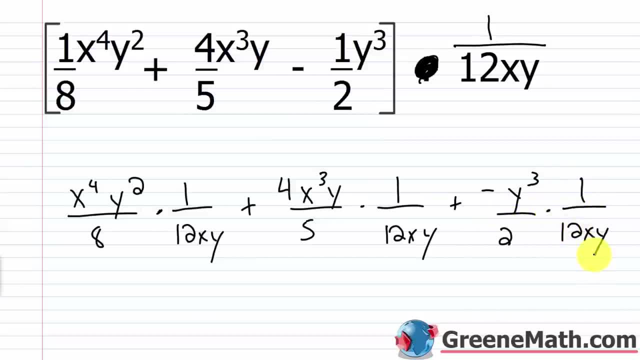 Over 2 and again times 1 over 12 x y 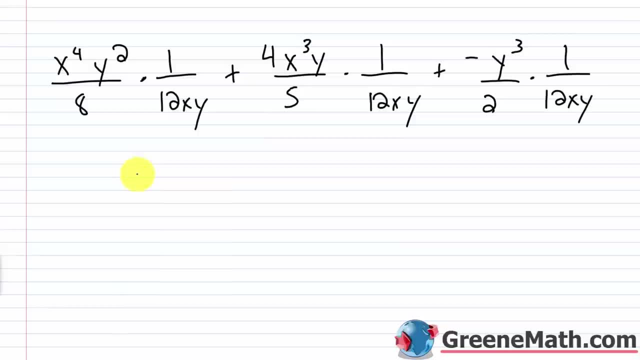 Alright so let's take a look at this now So what can we cancel Well here I'm cross canceling I can cancel one of the factors of x This will be x cubed With this x here I can cancel one of the factors of y This will be y to the first power And then nothing else I can really do So in the numerator I'm going to have x cubed y In my denominator I'm going to have 8 times 12 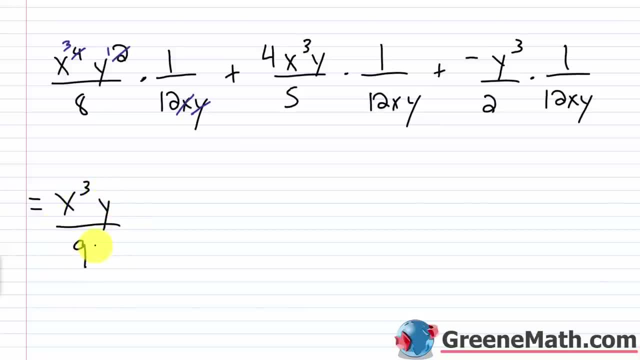 Which is 96 Then moving on to this part here I can easily see that 4 we cancel with 12 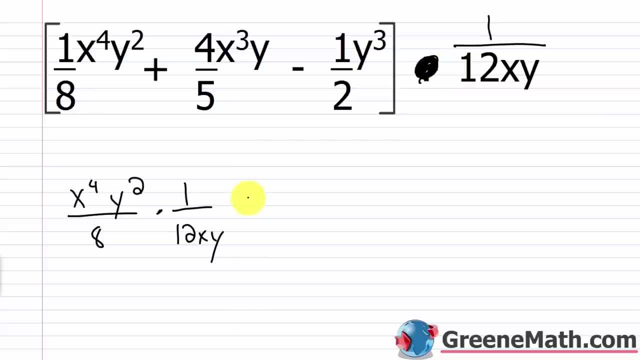 it's just going to put you one step ahead. All right, then plus, We have 4x cubed, y over 5 times 1 over 12xy. Then we have minus. When I'm going to put plus negative, we have y cubed or you can put one y cubed. 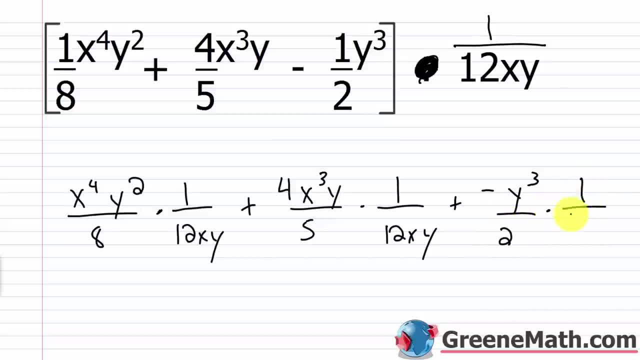 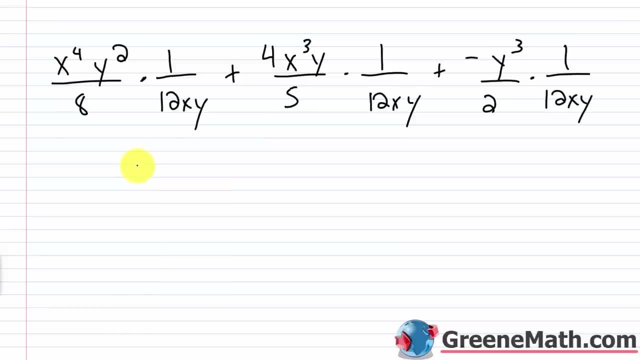 doesn't matter- over 2, and again, times 1 over 12xy. All right, so let's take a look at this now. So what can we cancel? Well, here I'm cross-canceling, I can cancel one of the factors of x. 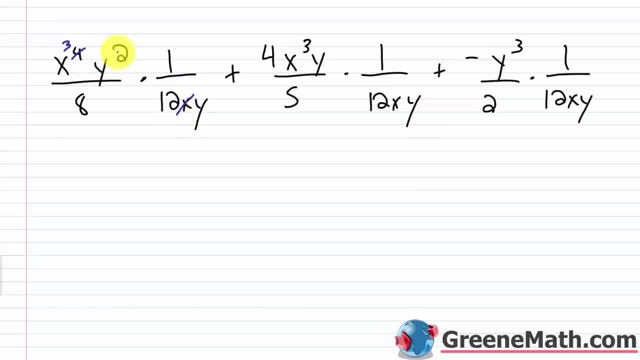 This will be x cubed with this x. here I can cancel one of the factors of y. This will be y to the first power with this y And then nothing else. I can really do So in the numerator I'm going to have x cubed y. 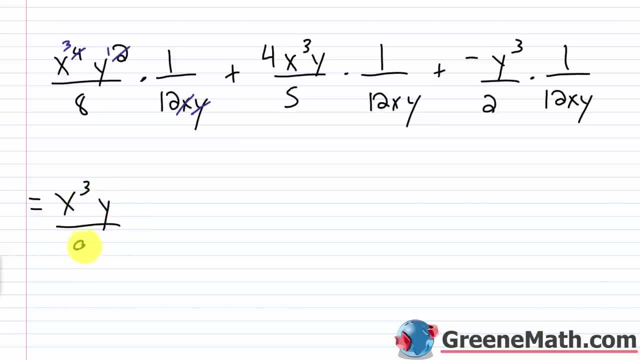 In my denominator I'm going to have 8 times 12, which is 96.. Then, moving on to this part, here I can easily see that 4 would cancel with 12 and leave me a 3 down here, One of the factors from x cubed. we cancel with this x. here This would be x squared. 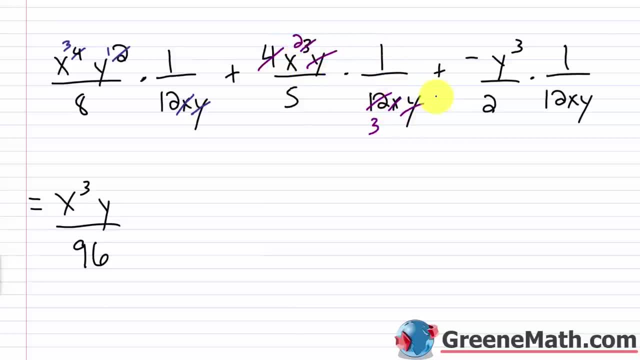 y, we cancel with y, So I would have x squared over 5 times 3, or 15.. So this is plus x squared over 15.. And then, for the last part, here I have y cubed over y. So one of the factors of y, 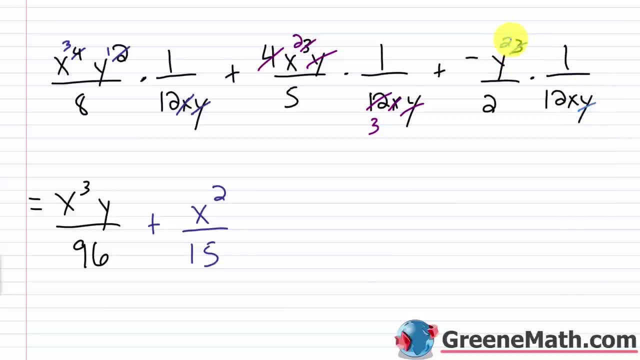 cubed would cancel with this, So this would be y squared And then nothing else I can really cancel. So you'd have negative y squared. I could put minus y squared over 2 times 12 is 24, and then times x, So 24x. So this is what we end up with as our answer. 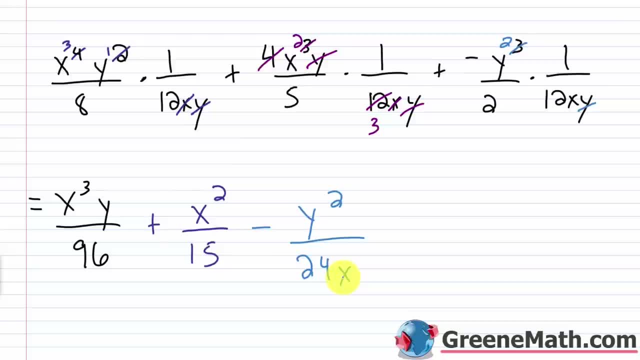 x cubed y over 96, plus x squared over 15, minus y squared over 24x. And again, if you want to check this, take your answer here. multiply it by the divisor. Remember when we started out, this problem was dividing by 12xy. So that's your divisor. 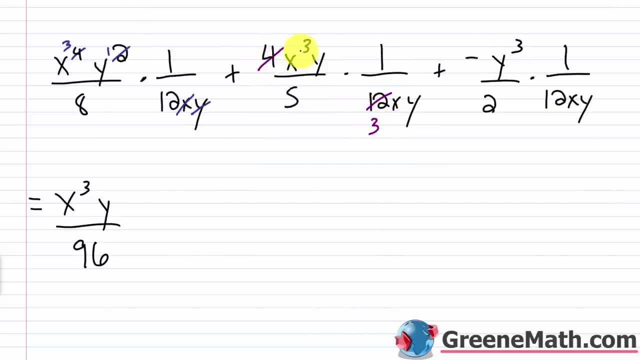 And leave me a 3 down here One of the factors from x cubed We cancel with this x here This would be x squared Y we cancel with y Over 5 times 3 or 15 So this is Plus x squared Over 15 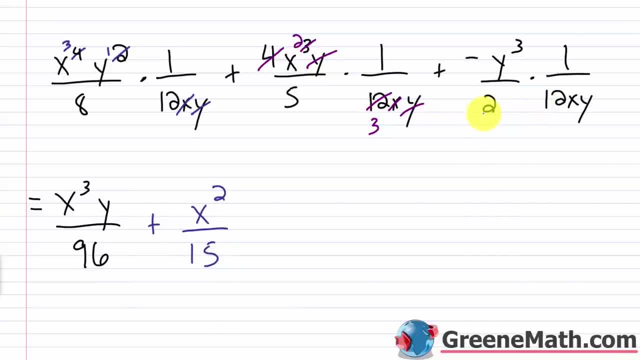 And then for the last part here I have 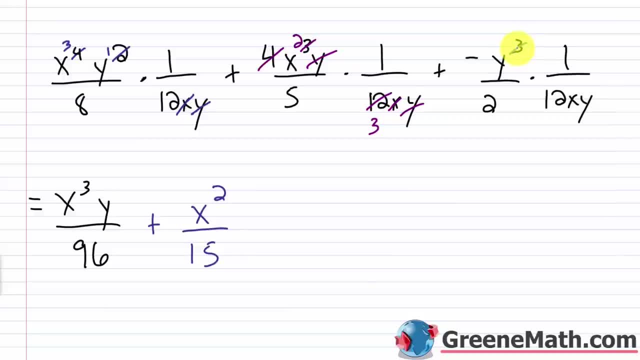 Y cubed over y So one of the factors of y cubed Would cancel with this So this would be y squared And then nothing else I can really cancel So you'd have negative y squared Or I could put minus Y squared over 2 times 12 is 24 And then times x So 24x So this is what we end up with as our answer 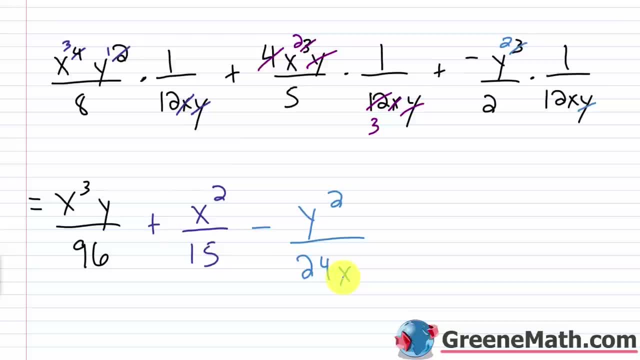 x cubed y over 96 Plus x squared over 15 Minus y squared over 24x 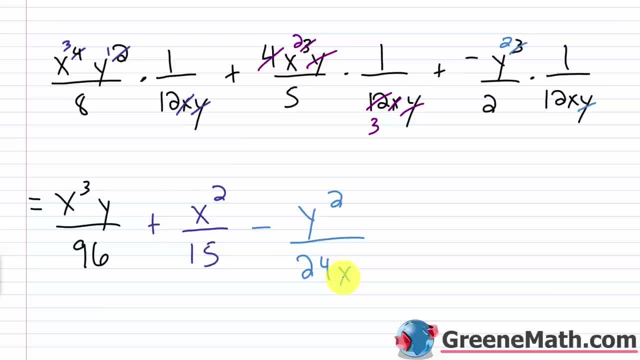 And again If you want to check this Take your answer here Multiply it by the divisor Remember when we started out This problem was Dividing by 12xy So that's your divisor 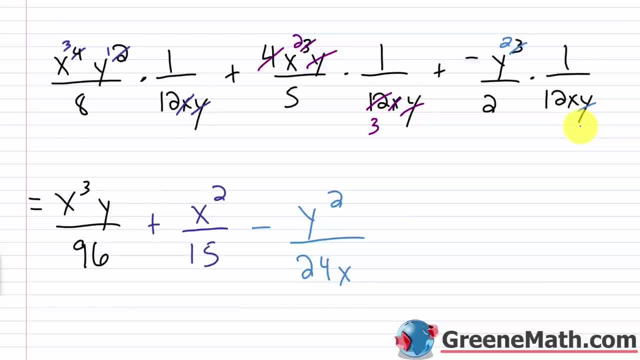 And again I modified it With fractions and it made it easier But when you do that You should get that original dividend back 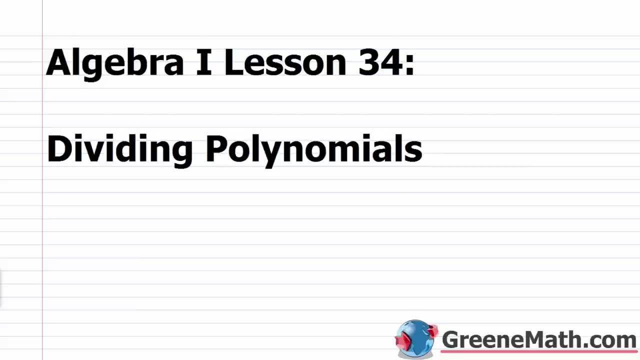 Hello and welcome to Algebra 1 Lesson 34 In this video we're going to learn about Dividing polynomials 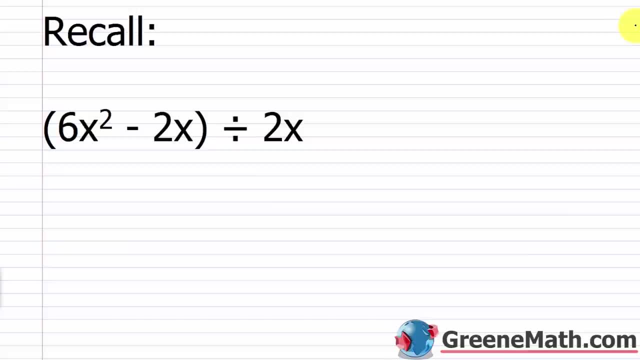 So in the last lesson we kind of got started With dividing polynomials We learned kind of the simplest case Where we divided a polynomial By a monomial So I want you to recall that if you had something like 6x squared minus 2x And we divided this by 2x Remember we could write this as a fraction 6x squared minus 2x Over 2x And then we could split this up Kind of using that same logic As when we work with fractions with whole numbers This is a common denominator 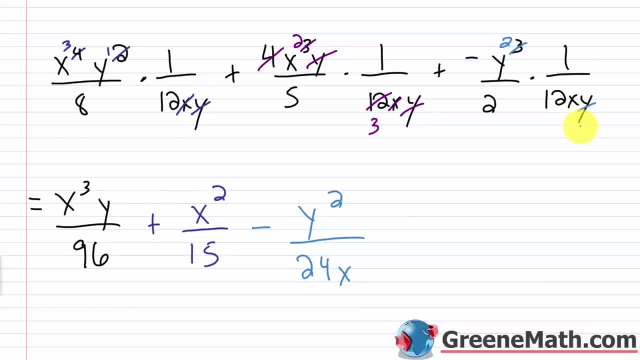 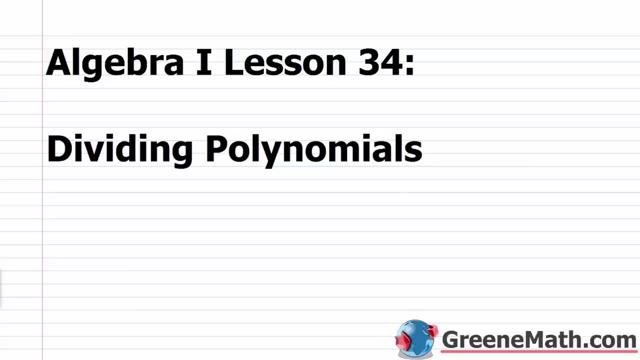 And again, I modified it just for the sake that we were working with fractions and it made it easier. But when you do that, you should get that original dividend back. Hello and welcome to Algebra 1, Lesson 34.. In this video, we're going to learn about dividing. 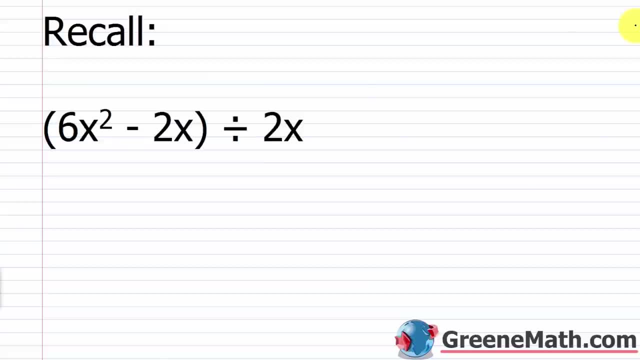 polynomials. So in the last lesson we kind of got started with dividing polynomials. We learned kind of the simplest case where we divided a polynomial by a monomial. So I want you to recall that if you had something like 6x squared minus 2x and we divided this by 2x. 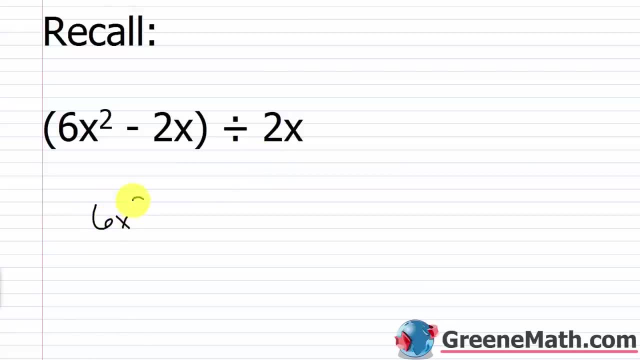 remember we could write this as a fraction, So 6x squared minus 2x over 2x, And then we could split this up right, kind of using that same logic as when we work with fractions with whole numbers. right, This is a common denominator, So we could say this is 6x squared over 2x. 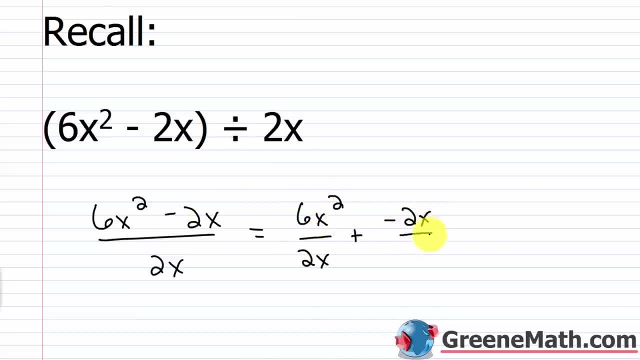 And then instead of minus I'm going to put plus, negative 2x over 2x. Then we can simplify each part separately. So 6 over 2 is 3.. x squared over x is just x to the first power. And then: 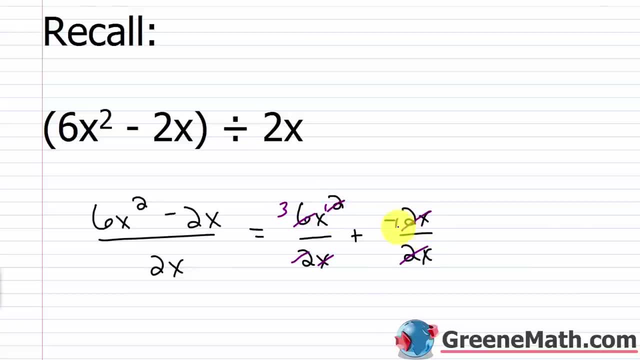 negative 2x, over 2x. this would just be negative 1.. So essentially, what I'd have here is 3x minus 1 as my answer. So let me write this as 3x minus 1.. Now another important thing: we know how to do. 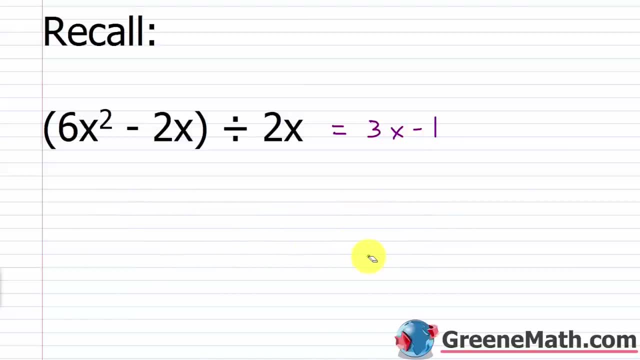 that at this point, Remember, if I want to check, I take the quotient, which is this guy, I multiply it by the divisor, which is this guy, and I should get the dividend back, which is this guy, So 2x. 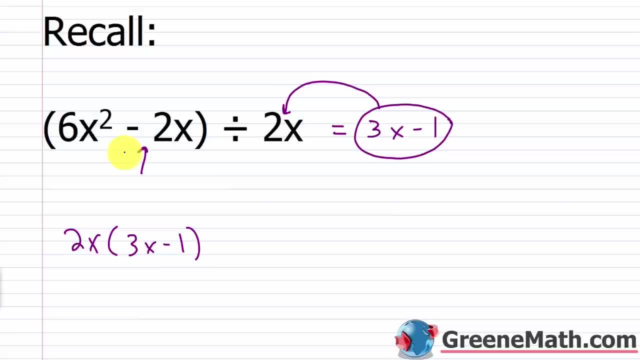 times 3x minus 1 should produce 6x squared minus 2x. So 2x times 3x is 6x squared, And then 2x times negative 1 is minus 2x. So we get that back exactly. 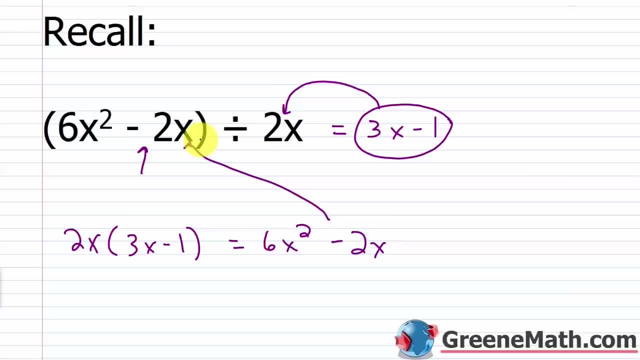 All right, so that's not very difficult. Hopefully you have mastered the concept of dividing a polynomial by a monomial. Once you've done that, it's really not much more difficult to divide a polynomial by a non-monomial polynomial, So in other words, a polynomial that 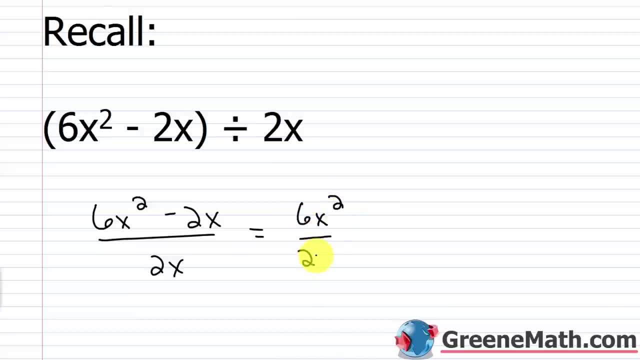 So we could say this is 6x squared over 2x And then instead of minus I'm going to put plus negative 2x Over 2x Then we can simplify each part separately So 6 over 2 is 3 x squared over x Is just x to the first power Over 2x this would just be negative 1 So essentially what I'd have here Is 3x minus 1 As my answer So let me write this as 3x minus 1 Now another important thing 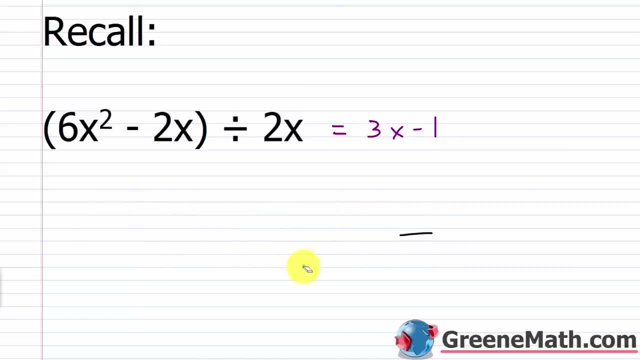 We know how to do that at this point Remember If I want to check I take the quotient which is this guy I multiply it by the divisor Which is this guy And I should get the dividend back Which is this guy So 2x times 3x minus 1 Should produce 6x squared minus 2x So 2x times 3x is 6x squared Then 2x times negative 1 is minus 2x So we get that back 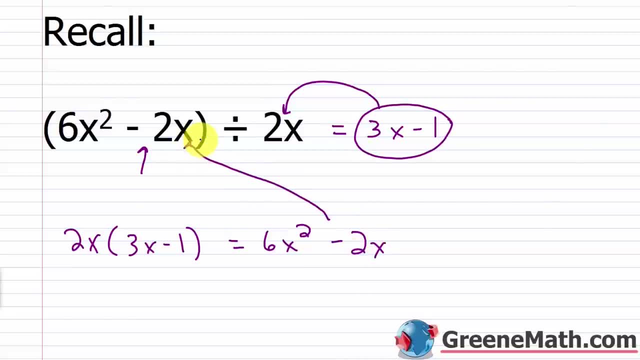 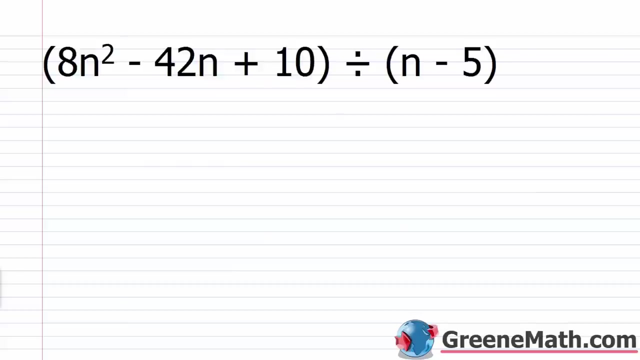 Exactly Alright so that's not very difficult Hopefully you have mastered the concept Of dividing a polynomial By a monomial Once you've done that It's really not much more difficult To divide a polynomial By a non-monomial polynomial So in other words a polynomial That consists of more than one term So for example if I saw something like 8n squared minus 42n Plus 10 And I divided this by n minus 5 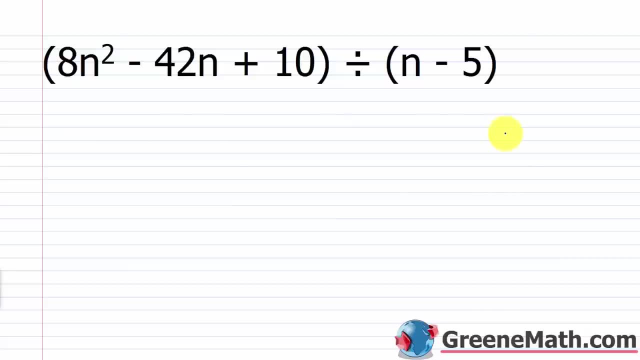 What would I do? Well I can't use the same technique That's not going to work anymore We need to turn to long division So the long division that we used With whole numbers We can use kind of a similar process For polynomials So let me just do a really really quick Rundown With long division of whole numbers That way it kind of refreshes your memory a little bit Let's say I had something like 4620 And I wanted to divide that by 5 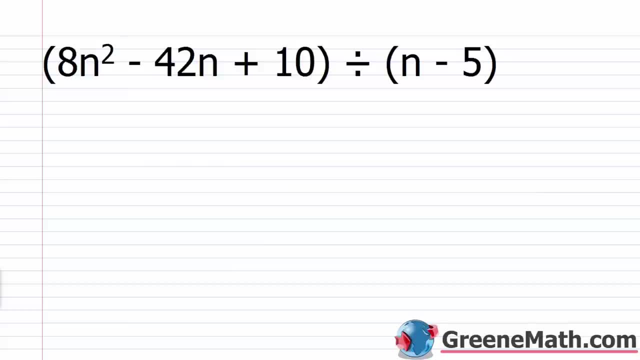 consists of more than one term. So, for example, if I saw something like 8n squared minus 42n plus 10, and I divided this by n minus 5,, what would I do? Well, I can't use the same technique. That's not going to work anymore. We need to turn to. 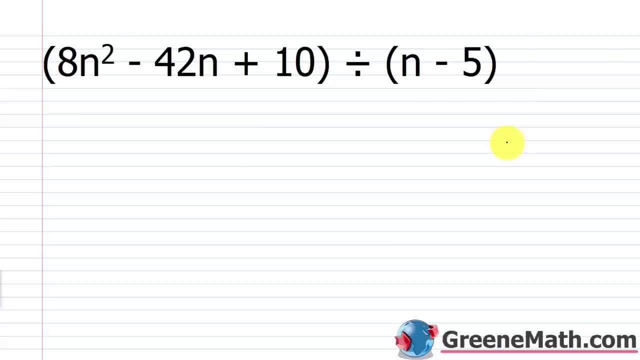 long division, right? So the long division that we used with whole numbers we can use kind of a similar process for polynomials. So let me just do a really really quick rundown with long division of whole numbers. That way it kind of refreshes your. memory a little bit. So let's do a really really quick rundown with long division of whole numbers. So let's do a really really quick rundown with long division of whole numbers. That way it kind of refreshes your memory a little bit. 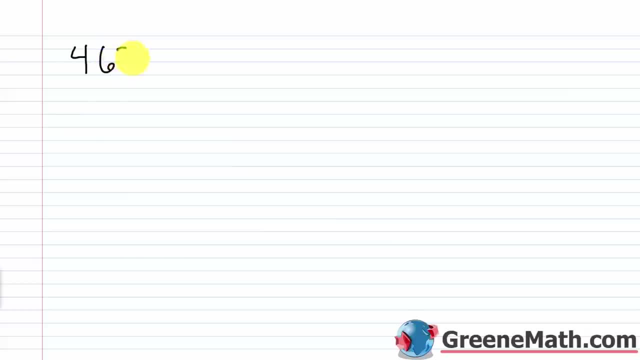 So let's do a really, really quick rundown with long division of whole numbers. That way it kind of refreshes your memory a little bit. Let's say, I had something like 4620, and I wanted to divide that by five. 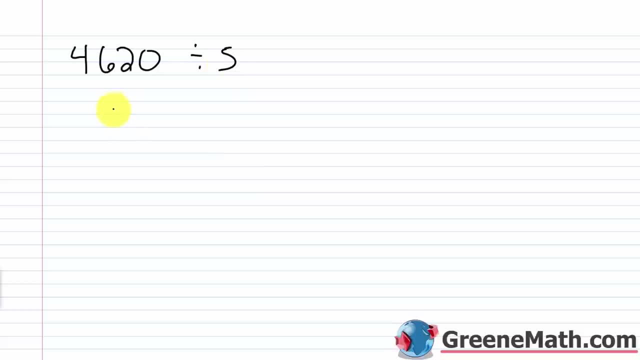 Remember the steps for long division. You're going to take your dividend, which is this number off to the left. This is the dividend, And you're going to start by putting that, as we say, under the house. So here's your 4620.. And then it's divided by five. The five is known as the divisor. 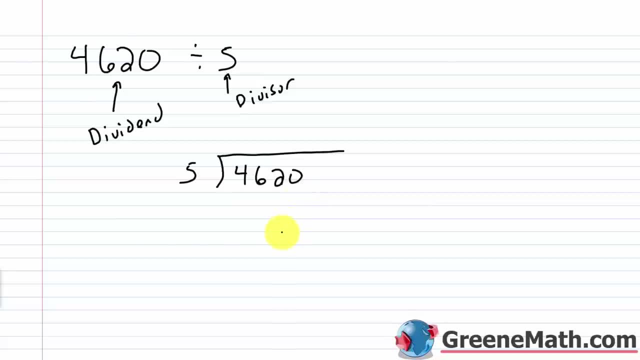 And that goes off to the left, And then it's divided by five, And then it's divided by five to the left. So once you have this set up, you recall we have that D which stands for divide, M which stands for multiply, S which stands for subtract, B which stands for bring down. 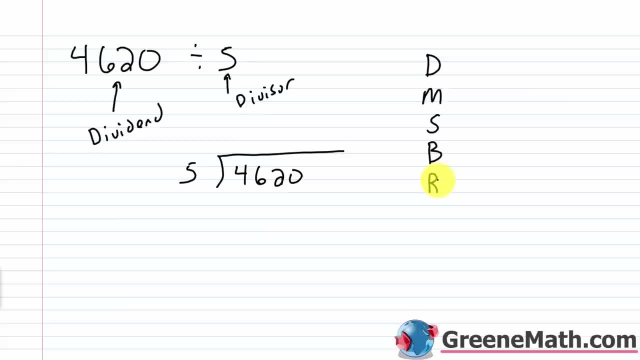 and then R, which stands for repeat or remainder. And the way you memorize this, you say dad, mom, sister, brother, rover right. You think about the family right, A mom and a dad, and then a brother and a sister and a family dog. So divide, multiply, subtract, bring down. 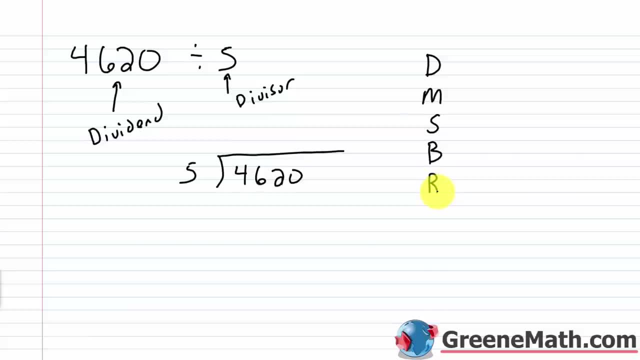 repeat or remainder. So when we get to polynomial division here in a second, it's going to be the same thing. There's a few slight differences, but basically we're following that format. So you start out by saying: how many times will five go into this leading term? four? Well, 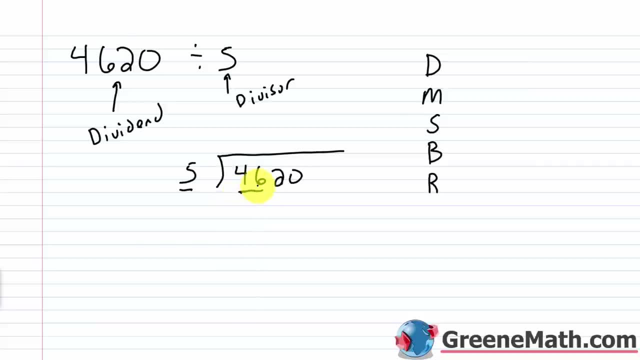 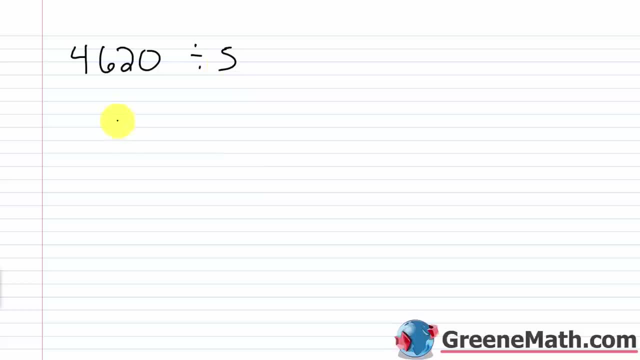 Remember the steps for long division You're going to take your Dividend Which is this number off to the left This is the dividend And you're going to start by putting that As we say under the house So here's your 4620 And then it's divided by 5 The 5 is known as the divisor And that goes off to the left So once you have this set up You recall we have that D which stands for divide 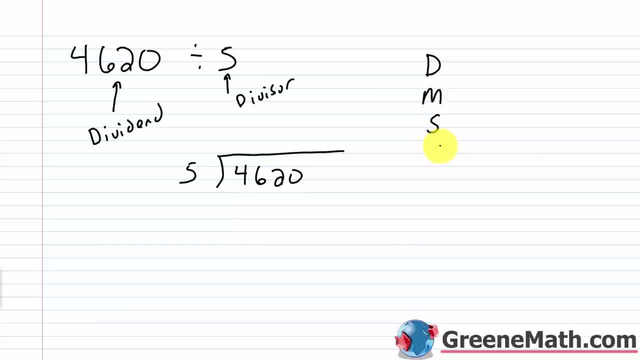 M which stands for multiply S which stands for subtract B which stands for bring down And then R which stands for repeat Or remainder And the way you memorize this You say dad, mom, sister, brother, rover You think about the family A mom and a dad and then a brother and a sister And a family dog So divide, multiply, subtract Bring down, repeat, or remainder 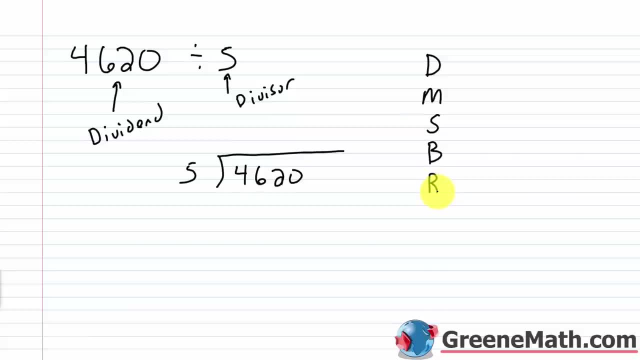 So when we get to polynomial division Here in a second It's going to be the same thing 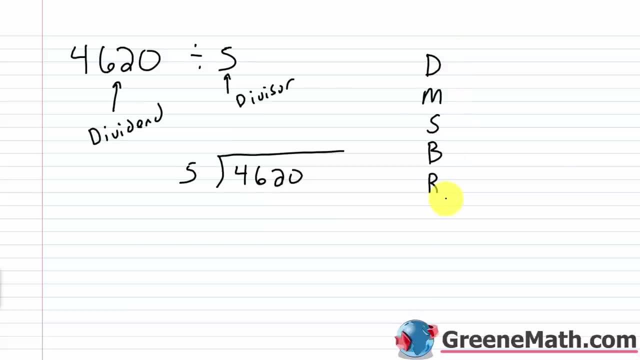 There's a few slight differences But basically we're following that format So you start out by saying How many times will 5 go into this leading term 4 Well it's not going to So what you do is You kind of expand that selection Say how many times will 5 go into 46 Well 5 will go into 46 9 times 9 times 5 is 45 Subtract and we get 1 So we did the division Then we multiplied Then we subtracted 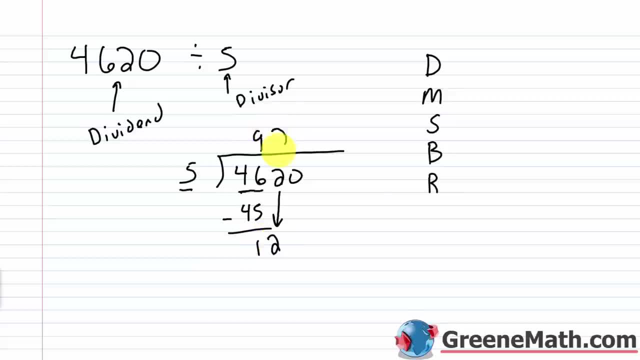 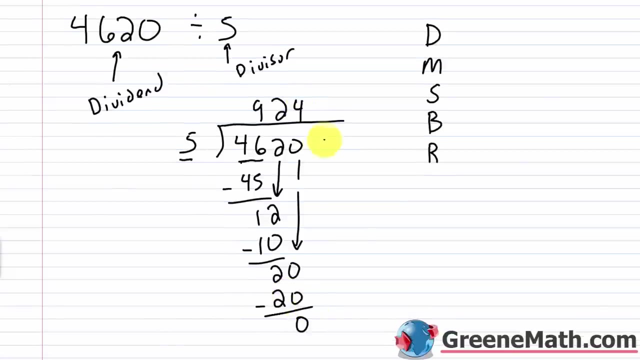 And now we just need to bring down So we bring down the 2 And then we repeat So 5 goes into 12 twice So we multiply 2 times 5 is 10 Subtract we get 2 Bring down We get 0 Nothing else to bring down So we're done So we get 924 as the result And that result is called the quotient 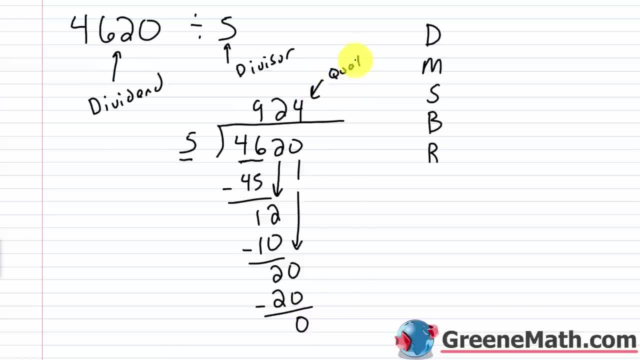 Let me label that That's called the quotient 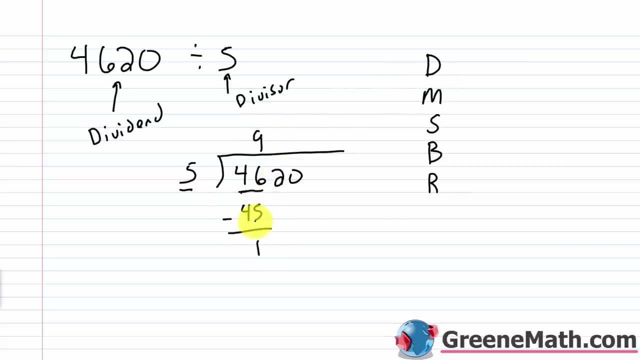 We get one. So we did the division, then we multiplied, then we subtracted and now we just need to bring down. So we bring down the two and then we repeat. So five goes into 12 twice. So we multiply Two times five is 10.. Subtract we get two, Bring down and then 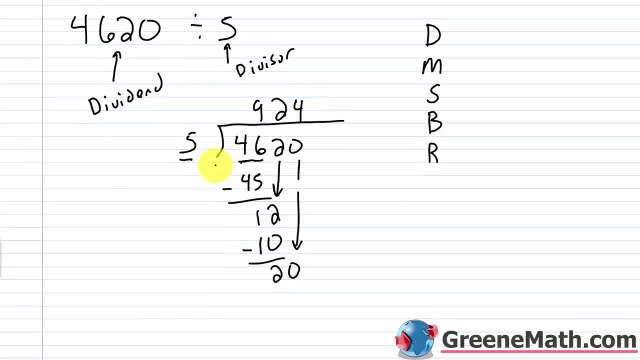 repeat. So now we divide again, Five goes into 24 times. Four times five is 20.. Subtract, we get zero. Nothing else to bring down, so we're done. So we get 924, as the result right, And that result is called the quotient. Let me label that. That's called the. 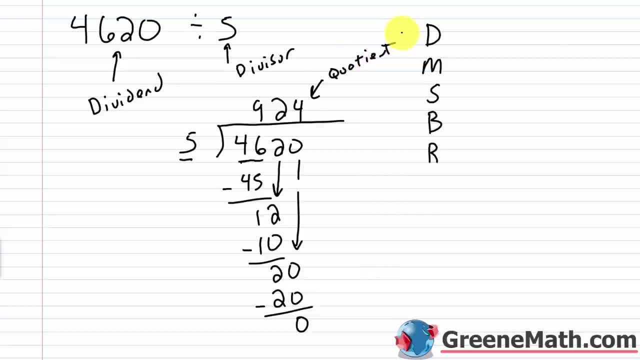 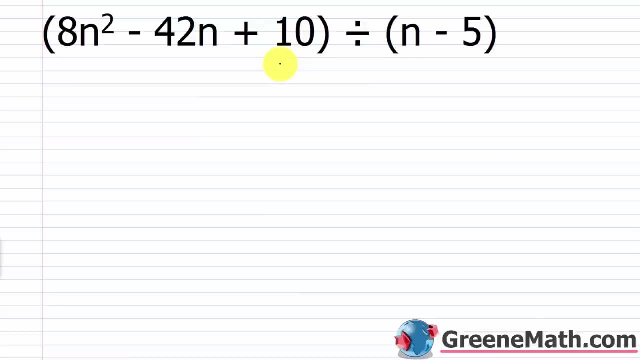 quotient. So we're going to follow a very similar process to divide polynomials. So go ahead and start out by setting this up in the same way that you did that long division problem with whole numbers. So again, this is your dividend and this is your divisor. So this goes under the house. So 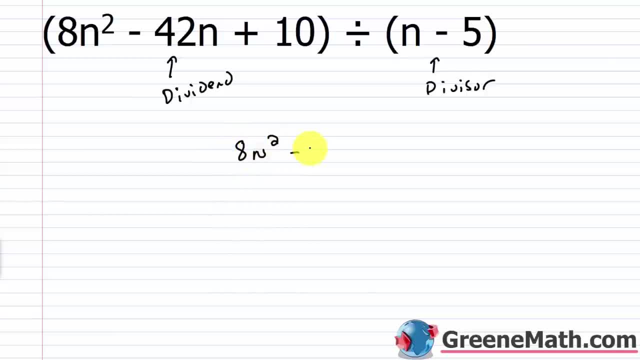 eight n squared minus 42n plus 10. And that goes under the house. And then, off to the left, we have n minus five. What's going to be different here? Remember your steps. You divide, you multiply. 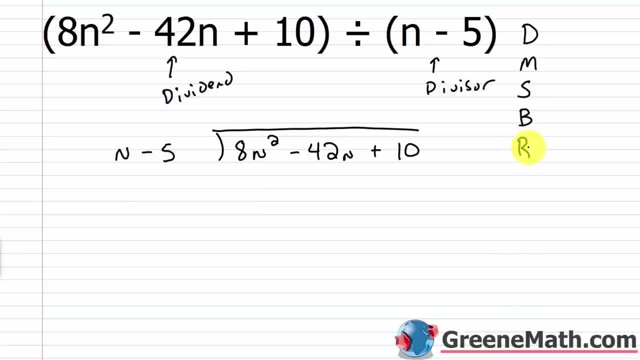 you subtract, you bring down and then repeat or remainder In the first step. here you're only thinking about the leading term of the divisor. So you're going to ask leading term of the divisor. So you're going to ask leading term of the divisor. 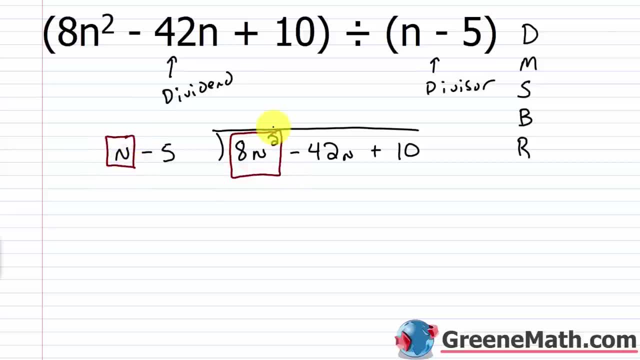 So you only want to know leading term into leading term. Okay, that's one of the differences. You're not including the minus five part there. Okay, so just forget about that. Now, what is this going to be? Well, it's just going to be 8n squared divided by n. That's all it is. You just need an answer to. 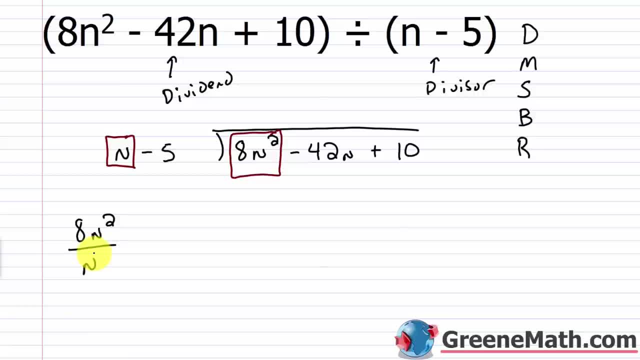 that question. So I always do that off to the side if I can't figure it out in my head. And it's easy to simplify this: We know that n squared over n would just be n to the first power. So this is 8n. So that's the answer. Now, just like with long division with whole numbers, I write my answer up. 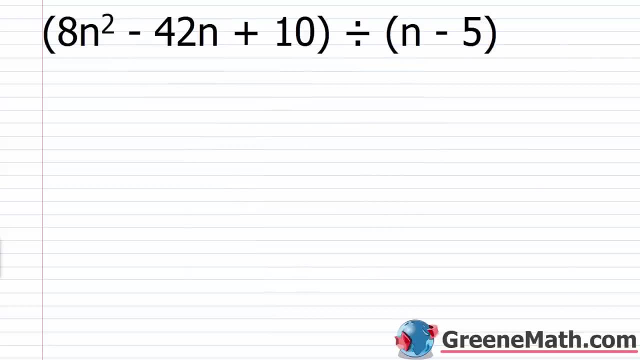 So we're going to follow a very similar process To divide polynomials So go ahead and start out by setting this up In the same way that you did That long division problem with whole numbers So again this is your dividend And this is your divisor So this goes under the house So 8 n squared Minus 42n Plus 10 And that goes under the house And then off to the left We have n minus 5 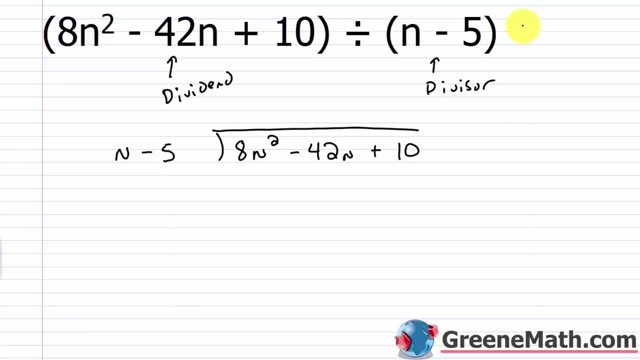 What's going to be different here Remember your steps You divide You multiply You subtract You bring down And you divide So here you're only thinking about The leading term of the divisor So you're going to ask Leading term into leading term So you only want to know Leading term into leading term That's one of the differences You're not including the minus 5 part 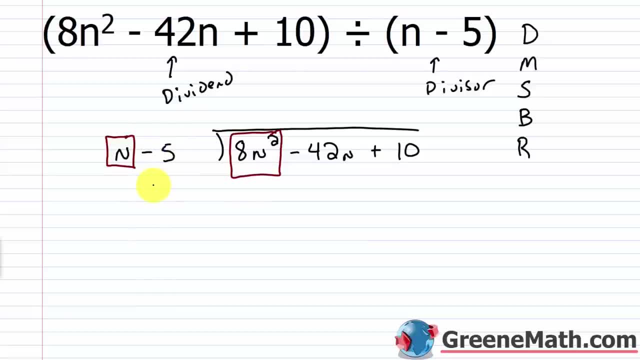 Just forget about that Now What is this going to be 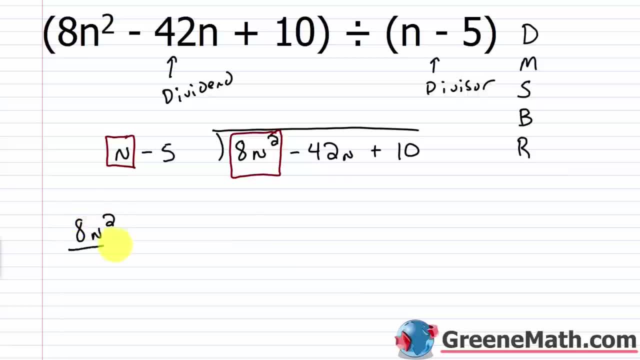 Well it's just going to be 8 n squared Divided by n 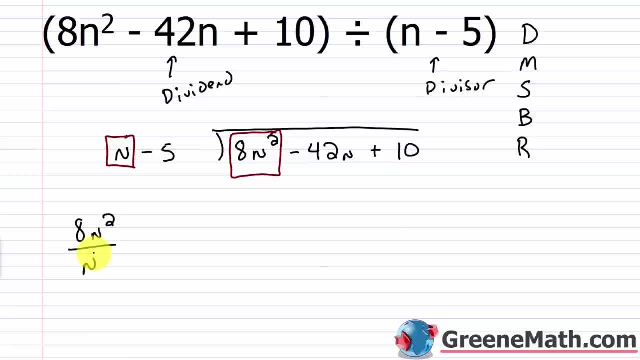 answer to that question. So I always do that off to the side if I can't figure it out in my head. 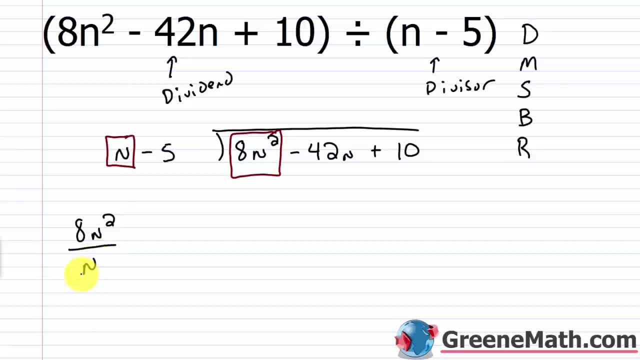 And it's easy to simplify this. We know that n squared over n would just be n to the first power, so this is 8n. So that's the answer. Now, just like with long division with whole numbers, I write my answer up here. But here's the main mistake that a lot of people make, and it's not that big of a deal, but I see a lot of students that will put 8n right here. It doesn't go there because you have to think about place value. This is where n squared goes, this is where n to the 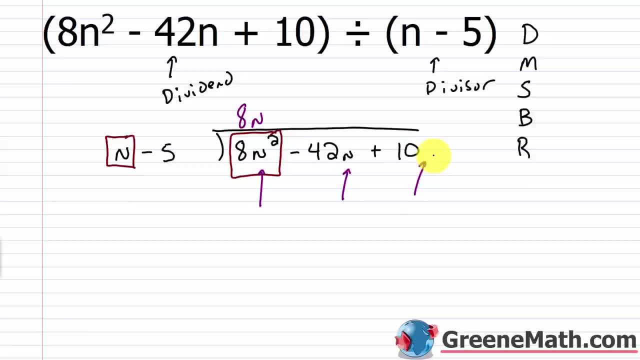 first power goes, and this is where n kind of to the power of zero or just a constant would go. 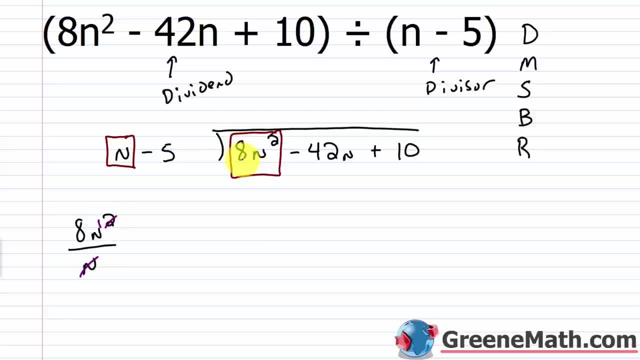 here. But here's the main mistake that a lot of people make. And it's not that big of a deal, But I see a lot of students that will put 8n right here. It doesn't go there because you have to think about place value. This is where n squared goes. This is where n to the first power goes. 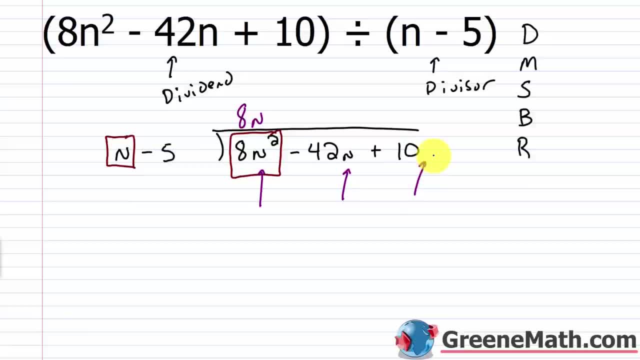 And this is where n kind of to the power of zero or just a constant would go. So we have n to the first power. So I'm going to shift that over here. I'm going to write my answer right here. 8n to the. 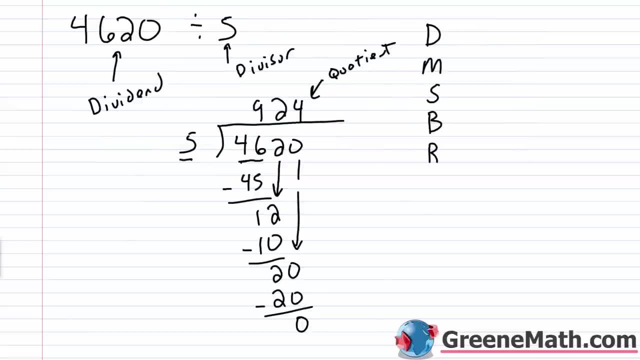 first power, And you can liken that to what we did here. I didn't write the nine all the way over here in front of the four, because this isn't 9,000, right, This is 900.. And so we want to. 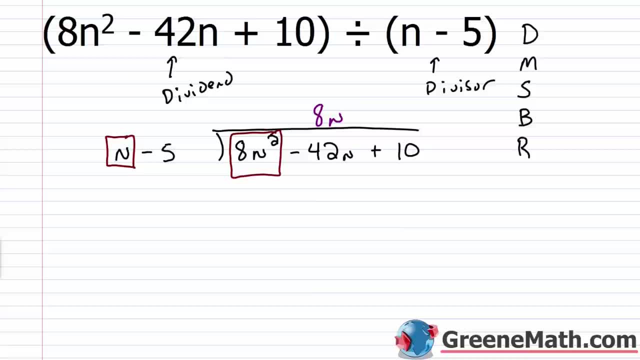 maintain place value, even though we're not working with whole numbers anymore. So this is kind of where n to the first power goes. So that's where I'm going to put the 8n when I get that as my answer. All right, So now I want to multiply. So 8n times n is 8n squared. 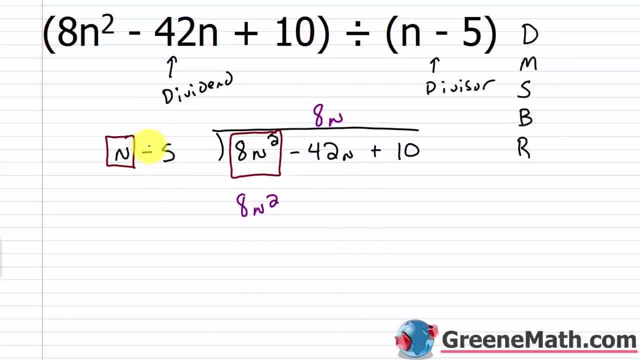 And I also want to multiply by the minus 5.. So 8n times negative, 5 is minus 40n. So that's the main thing to remember. Everything else is pretty much the same, because when I multiply, I multiply the 1 through 10. And then at the end I multiply by the minus 5.. So 8n times 2 minus 4 is minus 40n. 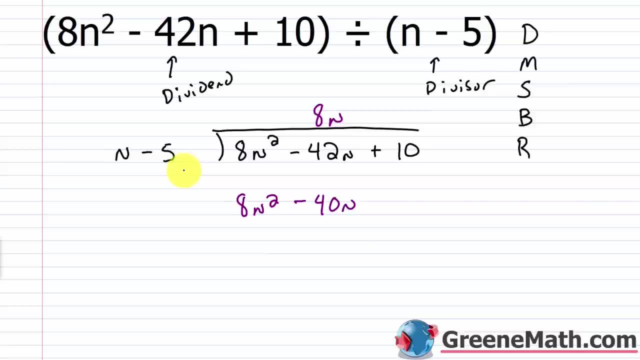 minus that, And so to get this in the model 1 plus 5, I have to divide by the 8n Milk Badge of N, And then 1,, 2,, 3, and so forth. I multiply thisOne part of by items 1, by items 3, by items is: 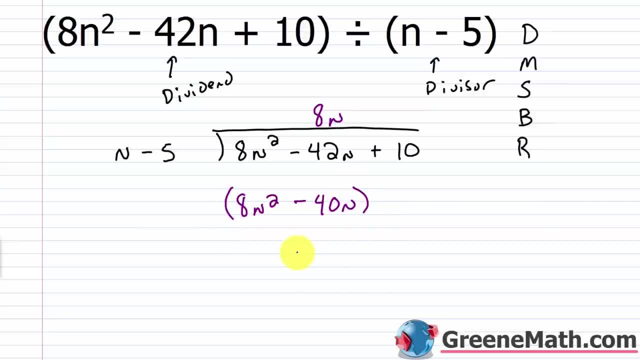 my N. So there is only one canvas of my어�guide total table with a scale and only two terms mean that you can actually multiply the simplify notes of the arrow keys byодарing the arrows And in the perspective, when I multiply by the knlil, the n girth of the n, I multiply by the subtract at n and possible. 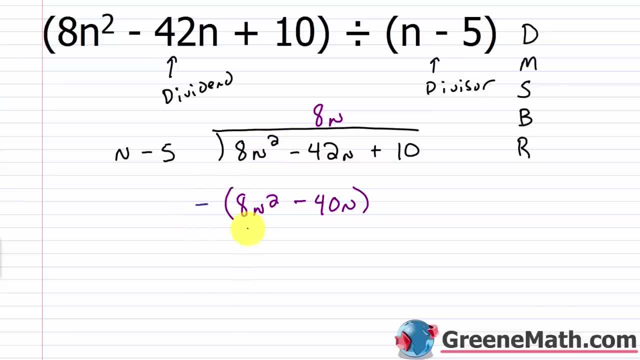 So it's just a little bit smaller than that. However, when we divide Yoga for both numbers three- and You can do it this way- you'll say 8n squared minus 8n squared is 0, negative 42n minus. 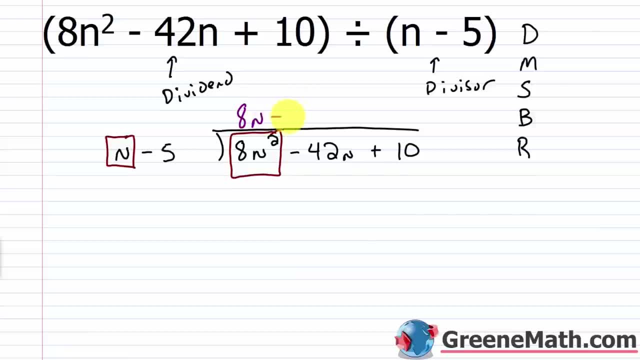 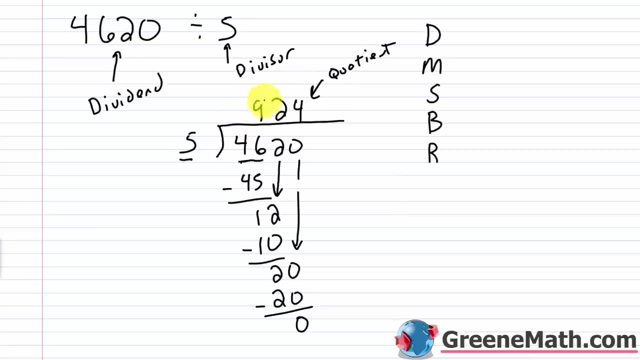 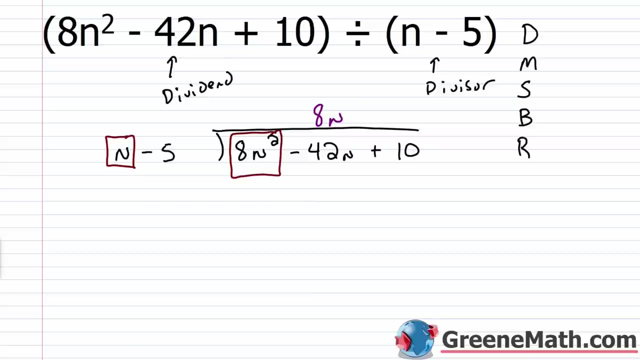 So we have n to the first power, so I'm going to shift that over here. I'm going to write my answer right here, 8n to the first power. And you can liken that to what we did here. I didn't write the 9 all the way over here in front of the 4 because this isn't 9,000, right? This is 900. And so we want to maintain place value even though we're not working with whole numbers anymore. So this is kind of where n to the first power goes, so that's where I'm going to put the 8n when I get that as my answer. All right, so now I want to multiply. So 8n times n is 8n squared. 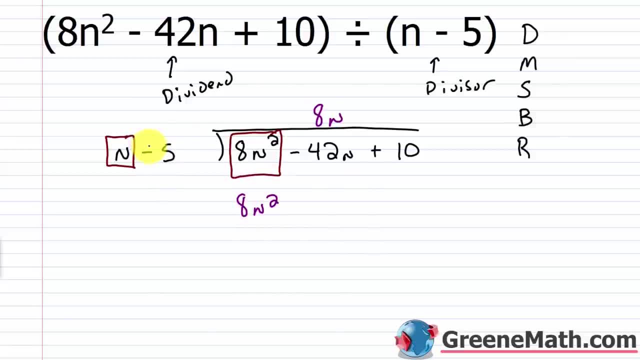 And I also want to multiply by the minus 5. So 8n times negative 5 is minus 40n. So that's the thing to remember. Everything else is pretty much the same because when I multiply, I multiply by everything. But when I do the division step, it's only leading term into leading term. So that's one of the things you just have to remember, and it's just one of those things you're just going to have to practice. And after you practice 10 or 15 of these, you're just going to remember. And then once I've done these two steps, the next step is to subtract. So I'm subtracting this whole thing away. Now, there's a few different ways to do this. What I always do and what I'm going to do in these videos is I'm going to subtract the whole thing away. So I'm going to subtract the whole thing away. 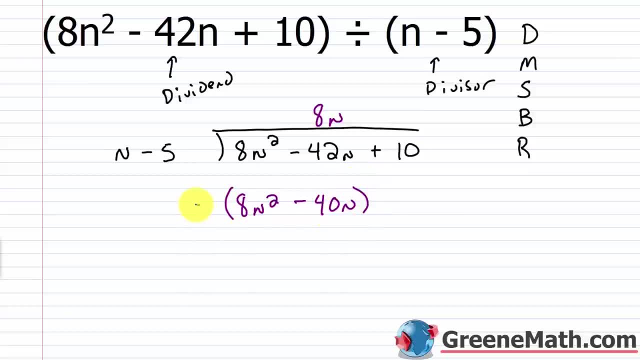 And what I'm going to do is I'm going to put parentheses around this guy, and I'm going to put a minus sign there. Now, you can do it this way. You'll say 8n squared minus 8n squared is 0, negative 42n minus a negative 40n. Minus a negative is plus a positive, so that would be negative 2n. You could do it that way. Or you can put a minus sign out front of these parentheses, and then you could just say, that's a reminder to remove the parentheses and to change the sign of each term. So this would be minus 8n squared. This would be plus 40n. And then I can add 8n squared minus 8n squared is 0, negative 42n plus 40n is negative 2n. You're going to get the same answer either way, so it doesn't matter how you want to do it. 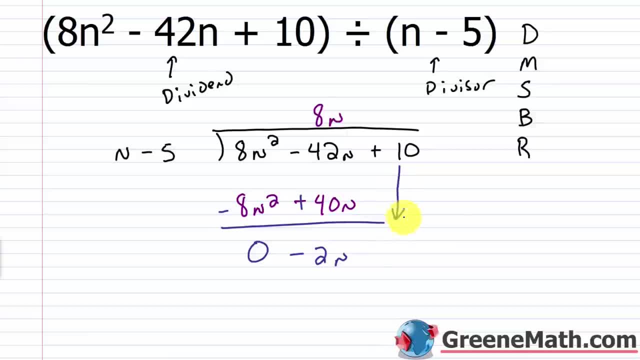 Then after the subtraction, we bring down. So plus 10. And now I can erase that 0. I don't need that. 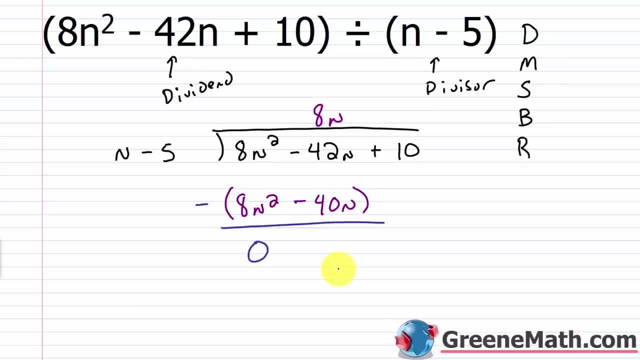 a negative 40n minus. a negative is plus a positive, so that would be negative 2n. you do it that way Or you can put a minus sign out front of these parentheses and then you could just say that's a reminder to remove the parentheses and to change the sign of each term. 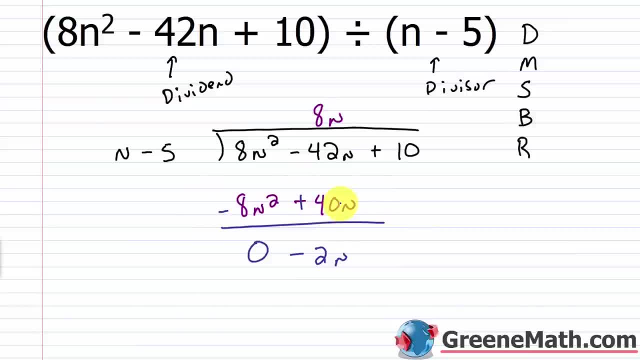 So this would be minus 8n squared, this would be plus 40n. and then I can add: 8n squared minus 8n squared is 0, negative 42n. plus 40n is negative 2n. You're going to get the same answer either way, so it doesn't matter how you want to. 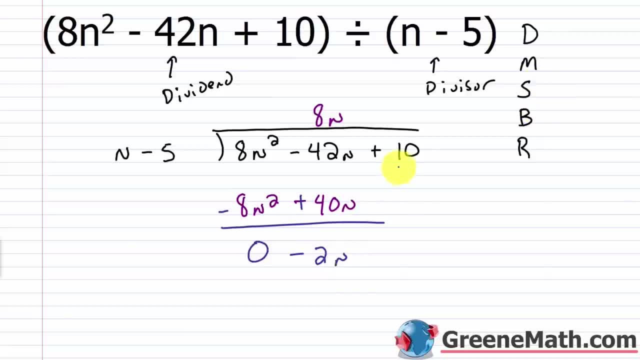 do it. Then after the subtraction we bring down So plus 10, and now I can erase that 0,. I don't need that Now. I can just do again the repeat step. So I go back up to the top. So it's leading term. 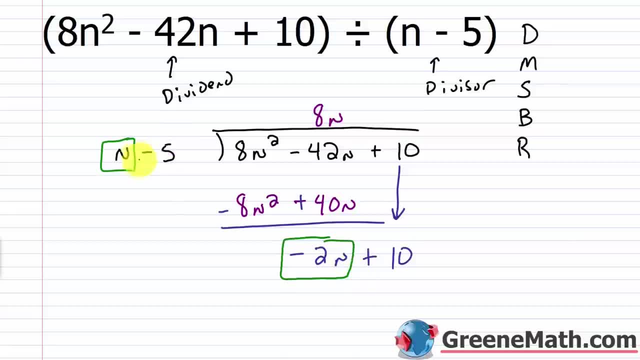 Into leading term. I'm not involving that negative 5 there. it's always just the leading term into the leading term. So what is negative? 2n over n? We know that the n's would cancel and I'm left with just negative 2.. 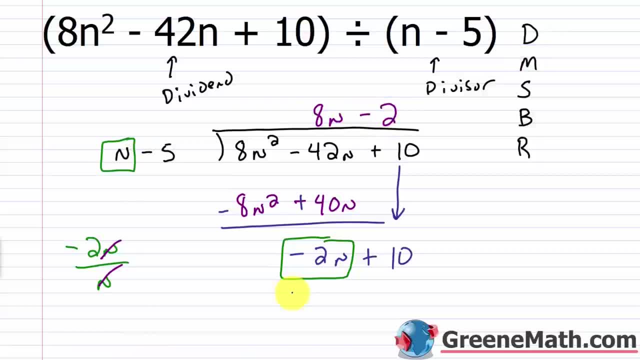 So negative 2 goes up here. then I multiply: negative 2 times n is negative 2n. negative 2 times negative 5 is plus 10.. Now we subtract, Now we know the same thing over itself is going to be 0.. 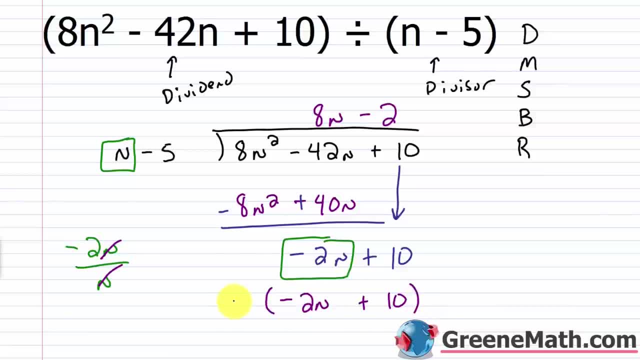 But for the sake of completeness, Let's go through and put parentheses around this guy and put a minus out in front. And then that reminds me, hey, I need to change the sign of each term. So this will be plus, this will be minus, and then I can erase this. 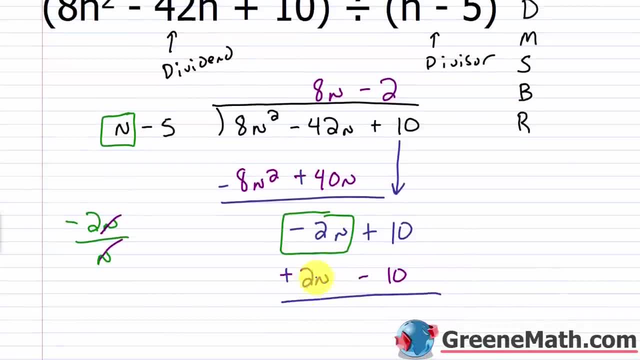 Just a reminder for me. So negative 2n plus 2n is 0,, 10 plus negative 10, or 10 minus 10 is 0. So I get a 0 there. Nothing else to bring down. So this 0 tells me that I don't have a remainder. 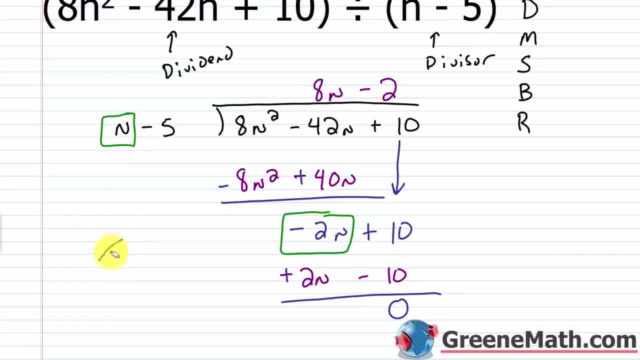 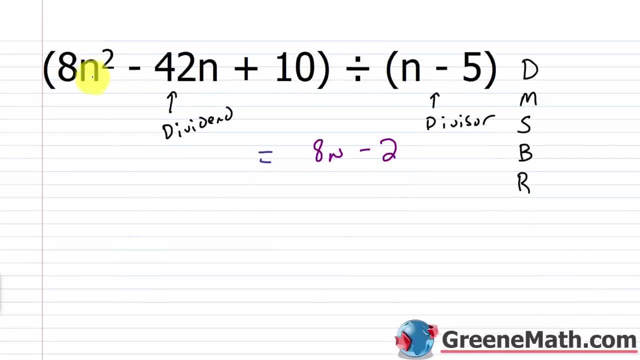 Now let's talk about something else. We know how to check division. When I have my answer, when I have my quotient, all I need to do is multiply it by the divisor. So this 8n minus 2 multiplied by n minus 5, and that should give me the dividend back. 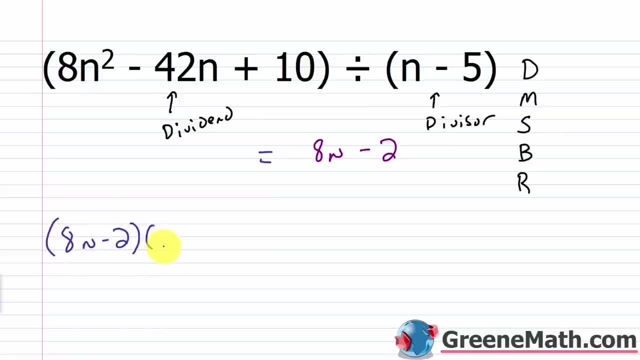 So 8n minus 2 multiplied by n minus 5, it only takes a second to check And you know if you're doing your homework and your homework's graded. why not get the right answer Right? So 8n times n is 8n squared. 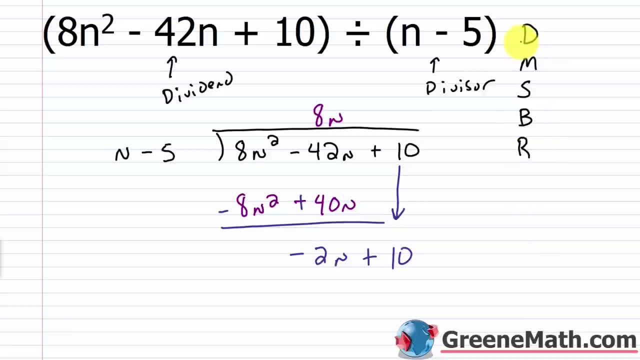 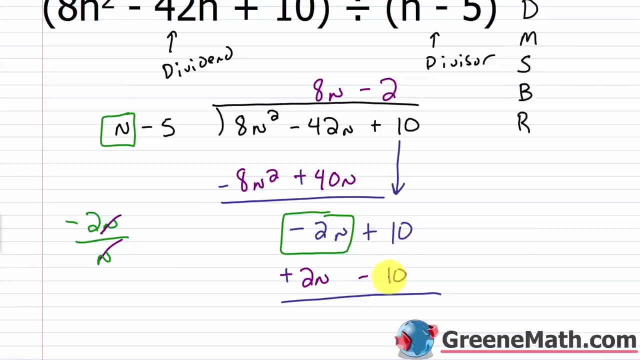 Now I can just do, again, the repeat step. So I go back to the previous step, and I'm going to do up to the top. So it's leading term into leading term. I'm not involving that negative 5 there. It's always just the leading term into the leading term. So what is negative 2n over n? Well, we know that the n's would cancel, and I'm left with just negative 2. So negative 2 goes up here. Then I multiply. Negative 2 times n is negative 2n. Negative 2 times negative 5 is plus 10. Now we subtract. Now we know the same thing over itself, it's going to be 0. But for the sake of completeness, let's go through and put parentheses around this guy and put a minus out in front. And then that reminds me, hey, I need to change the sign of each term. So this will be plus, this will be minus, and then I can erase this. Just a reminder for me. So negative 2n plus 2n is 0. 10 plus negative 10, or 10 minus 10 is 0. So I get a 0 there. Nothing else to bring down. So this 0 tells me that I don't have a remainder. Now, let's talk about something else. We know how to check division. 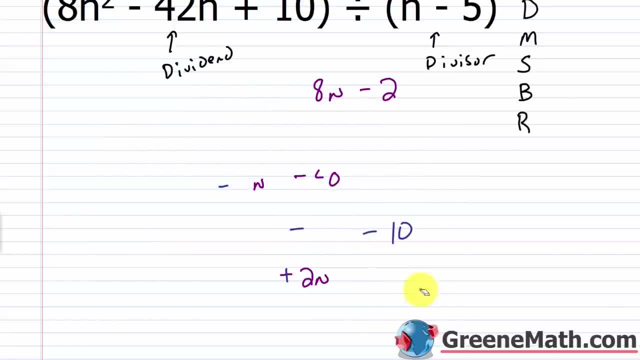 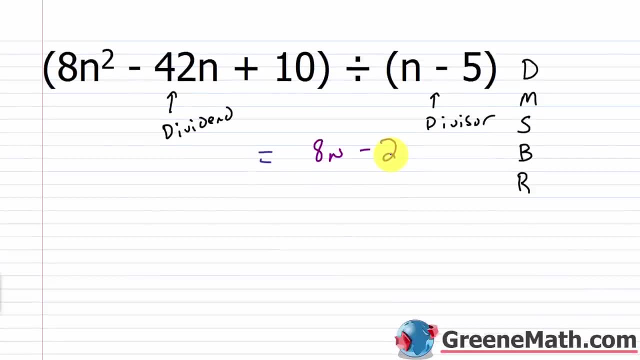 When I have my answer, when I have my quotient, all I need to do is multiply it by the divisor. So this 8n minus 2 multiplied by n minus 5, and that should give me the dividend back. So 8n minus 2 multiplied by n minus 5. It only takes a second to check. And you know, if you're doing your homework and your homework's graded, why not get the right answer, right? So 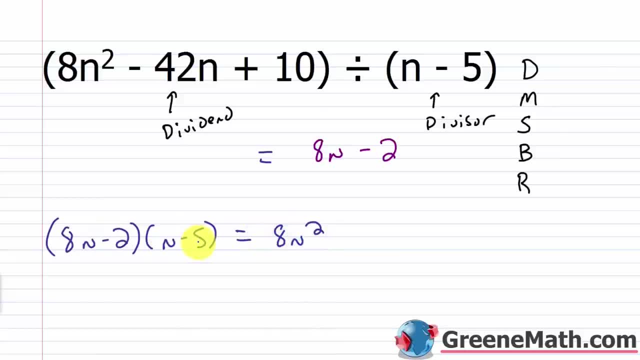 8n times n is 8n squared. Then 8n times negative 5 is minus 40n. Then negative 2 times n is negative 2n. Then negative 2 times negative 5 is plus 10. So this equals 8n squared. Negative 40n minus 2n is minus 42n. And then plus 10. So you can see we get exactly the dividend back. 8n squared minus 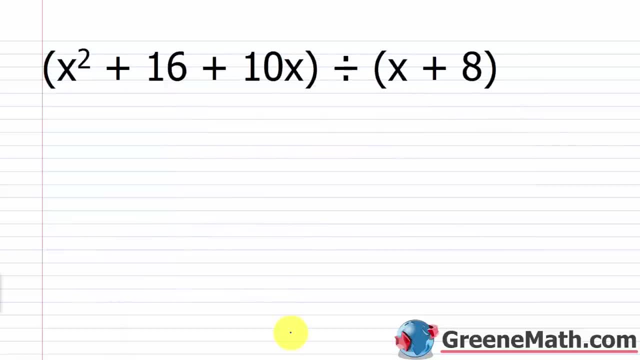 42n plus 10. All right, so that was pretty easy. Let's take a look at another one. So we have, 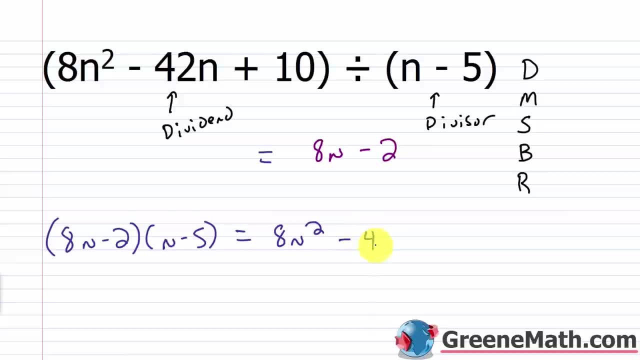 All right. So 8n times n is 8n squared. Then 8n times negative, 5 is minus 40n. Then negative 2 times n is negative 2n. Then negative 2 times negative, 5 is plus 10.. 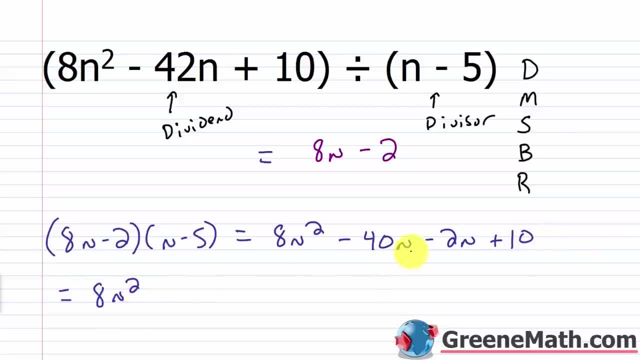 So this equals 8n squared negative. 40n minus 2n is minus 42n and then plus 10.. So you can see we get exactly the dividend back: 8n squared minus 42n plus 10.. 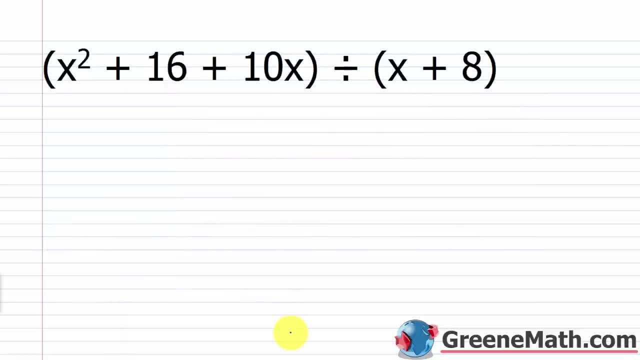 All right, So that was pretty easy. Let's take a look at another one. So we have x squared plus 16 plus 10x. All right, So we have x squared divided by x plus 8.. So one of the things I haven't mentioned yet is that each polynomial when you're doing 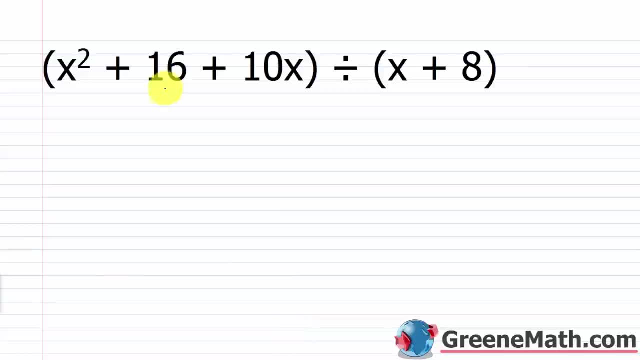 the division has to be in standard form. So this is out of order, right? The 10x should be over here, The 16 should be over here. So when I set this up in long division format, I'm going to correct that. 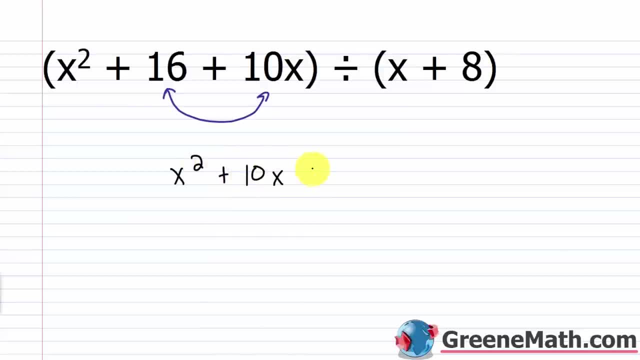 So I'm going to say I have x squared plus 10x plus 16, and this is divided by x plus 8.. All right. So if you see a polynomial that's not in standard form, you need to fix that. So, for example, if this would have been 8 plus x, I would have flipped that and made 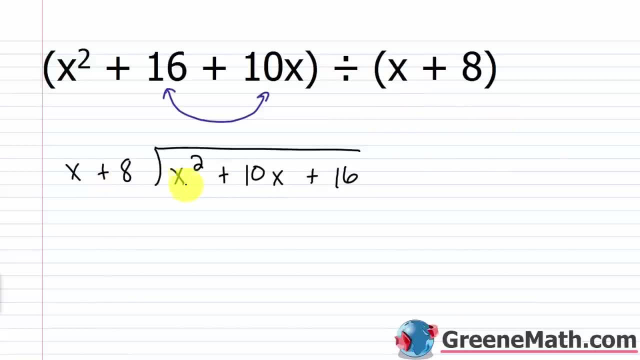 it x plus 8.. All right, So that's kind of the first thing you want to do when you're setting this up. Now we just go through the normal way, right? So let me write this down again: We have divide, multiply subtract, bring down, repeat or remainder, right? 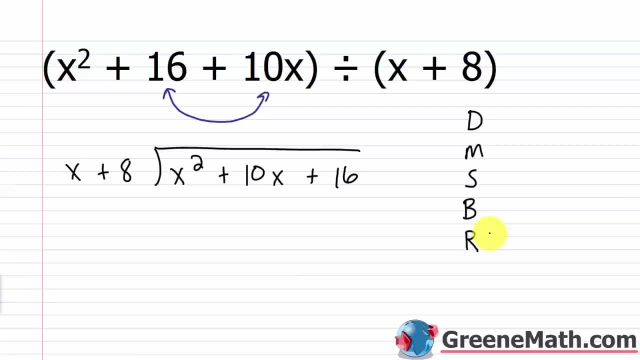 Dad, mom, sister, brother, rover. So again, I start out by saying leading term. All right, So I'm going to write down x squared plus 8 into leading term. okay, I'm not involving that plus 8, okay. 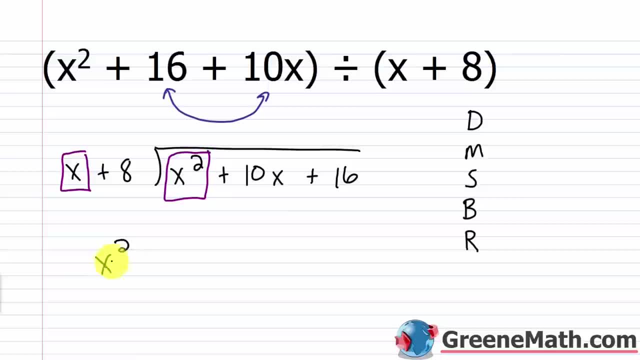 Not doing that. So what is x squared over x? We know that one of these would cancel with this and I just have x to the first power. Again, this is the spot for x squared. This is the spot for x to the first power. 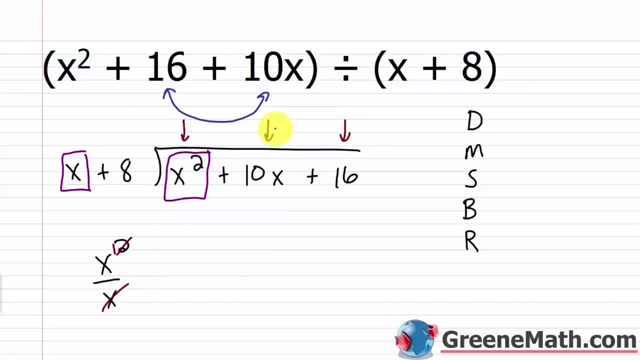 This is the spot for a constant. So we're going to put our answer here, because it's x to the first power, So that's going to go right there. Then we're going to multiply. Remember, when I multiply, I multiply by everything. 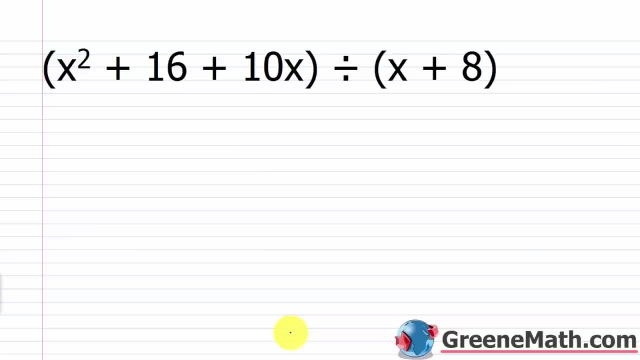 x squared plus 16 plus 10x divided by x plus 8. So one of the things I haven't mentioned yet is that each polynomial, when you're doing the division, has to be in standard form. So this is out of order, right? The 10x should be over here. The 16 should be over here. So when I set this up in long division format, I'm going to correct that. So I'm going to say I have x squared plus 10x plus 16. 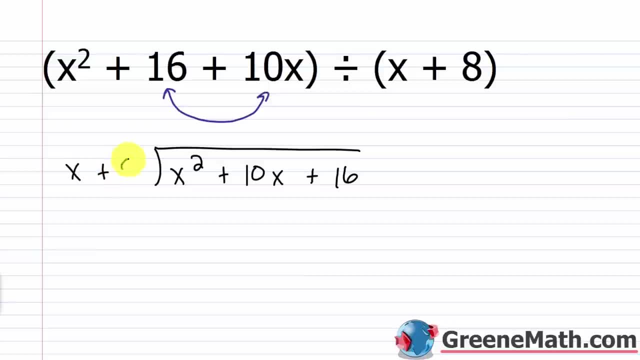 And this is divided by x. Plus 8. So if you see a polynomial that's not in standard form, you need to fix that. So for example, 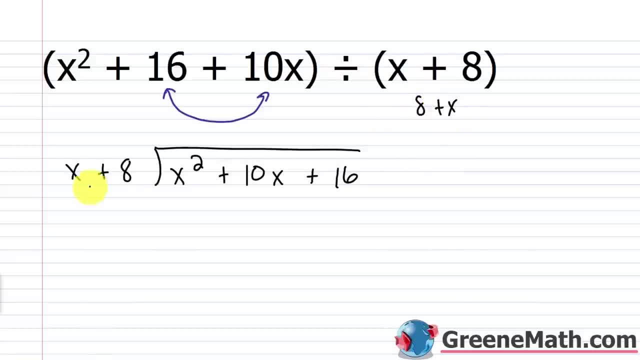 if this would have been 8 plus x, I would have flipped that and made it x plus 8. All right, so that's kind of the first thing you want to do when you're setting this up. Now, we just go 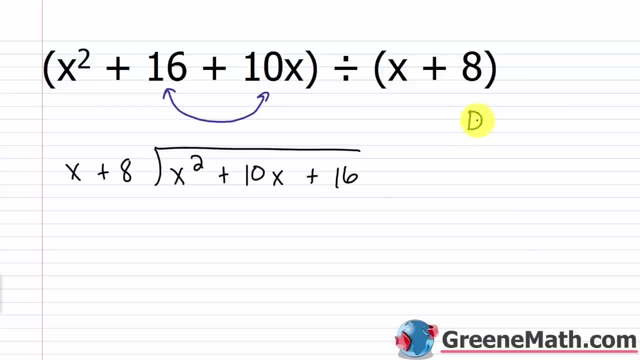 through the normal way, right? So let me write this down again. We have divide, multiply, subtract, bring down, repeat, or remainder, right? Dad, mom, sister, brother, rover. So again, I start off with a number. So I'm going to write this down. So I'm going to write this down. So I'm going to write this down by saying leading term into leading term, okay? I'm not involving that plus 8, okay? Not doing that. So what is x squared over x? We know that one of these would 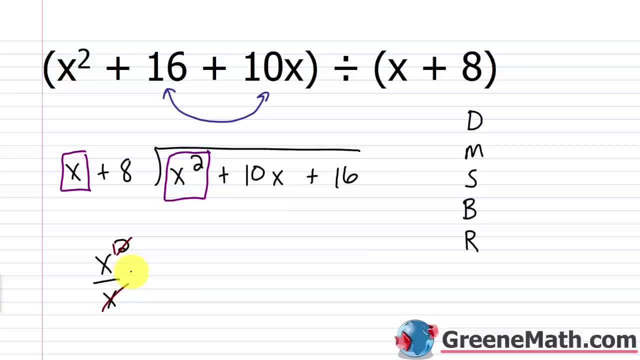 cancel with this, and I just have x to the first power. Again, this is the spot for x squared. This is the spot for x to the first power. This is the spot for a constant. So we're going to put our answer here because it's x to the first power. So we're going to put our answer here because it's x to the first power. 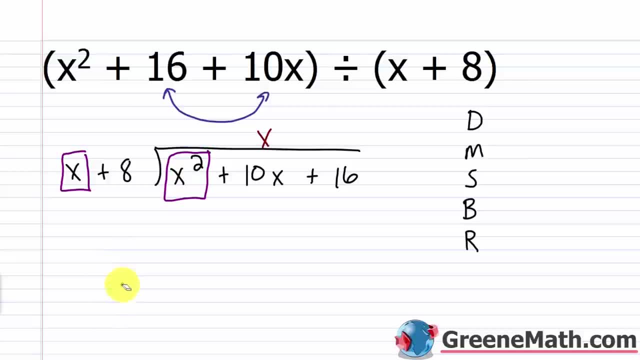 So that's going to go right there, and then we're going to multiply. Remember, when I multiply, I multiply by everything. So x times x is x squared. x times 8 is plus 8x, and then I subtract. 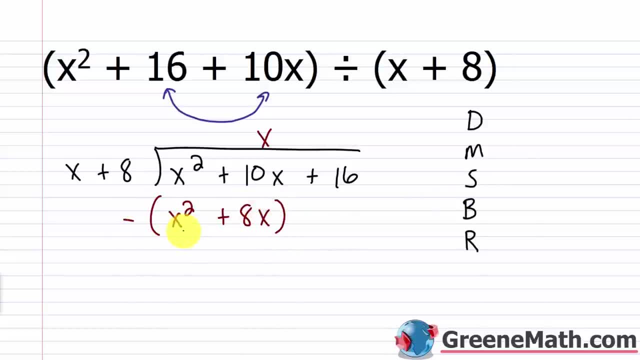 I subtract this guy away. Now, you do it like that, or again, use this as a reminder to put a minus here and a minus here, and then you can remove all the parentheses, and you can add. Either way, you want to do it. x squared minus x squared is 0. 10x minus 8x is 2x. 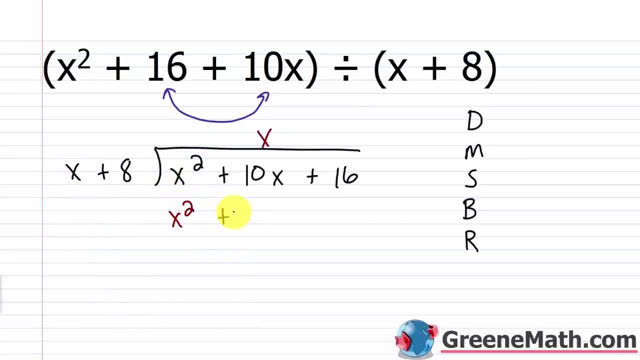 So x times x is x squared, X times 8 is plus 8x. And then I subtract. I subtract this guy away. Now you do it like that, or again use this as a reminder to put a minus here and a minus. 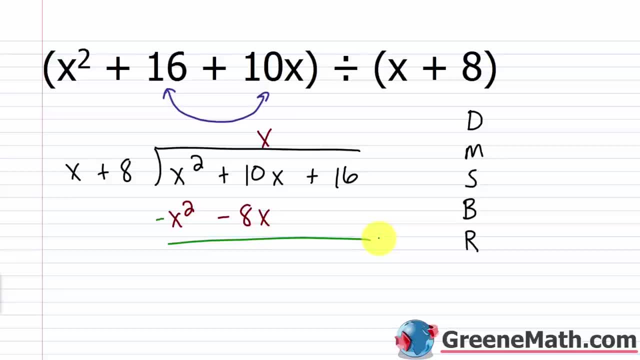 here, and then you can remove all the parentheses and you can add, Either way you want to do it: X squared minus x squared is zero. 10x minus 8x is 2x. Now we're going to bring this here. 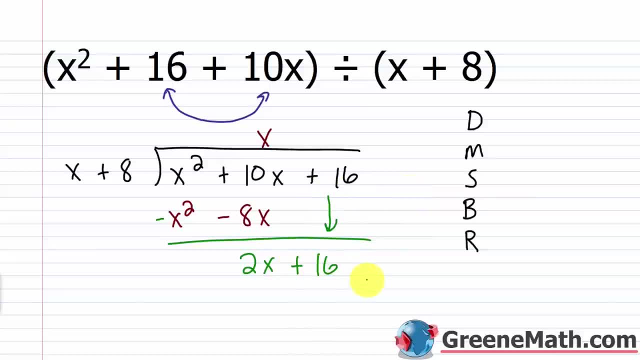 All right down, So plus 16.. And then we're going to repeat, So we go back up to the top, So we're going to go leading term into leading term. So what is 2x over x? Well, the x's would cancel and I would. 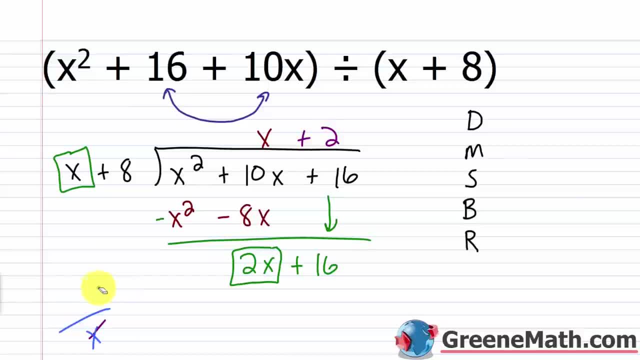 just have a 2.. So plus 2.. Again, multiply 2 times x is 2x. 2 times 8 is plus 16.. So we could see we wouldn't have a remainder here, right? Anything minus itself is 0. But again, for the sake of. 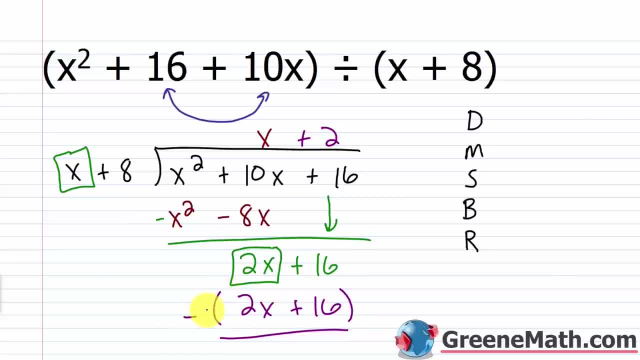 completeness. we're going to subtract this away, So I'm going to change the sign of each term. This will be minus And that'll be minus, And I can erase this. 2x minus 2x is 0.. 16 minus 16 is 0.. 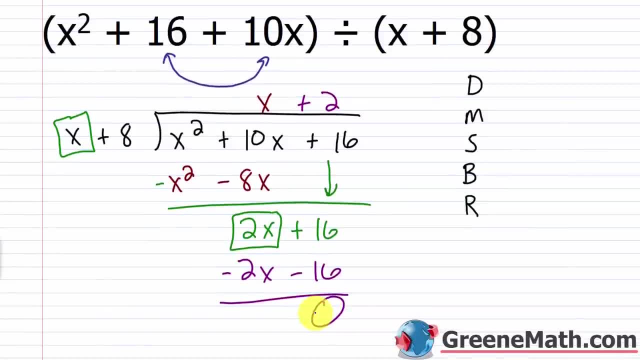 So again, there's no remainder. So our answer here is x plus 2.. So x plus 2.. And it's very, very easy to check. So again, if I wanted to take the quotient x plus 2 and multiply that by the, 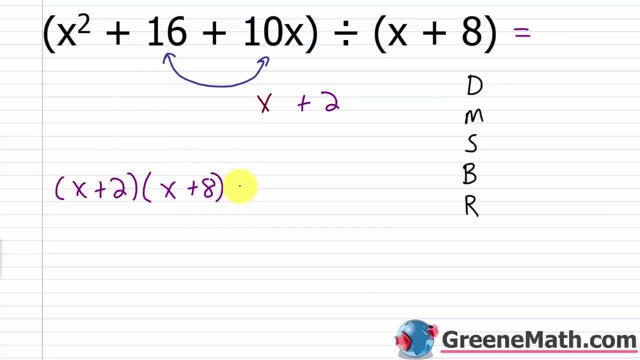 divisor x plus 8, I should get my dividend back. x times x is x squared. x times 8 is plus 8x. 2 times x is plus 2x. 2 times 8 is plus 16.. So if I combine like terms, 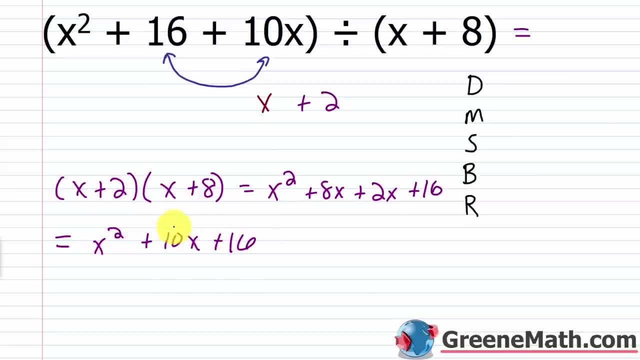 I get x squared plus 10x plus 16, which is exactly this. It just looks a little different because this is not in standard form and this is right. But if I flip the position here of the 10x and the, 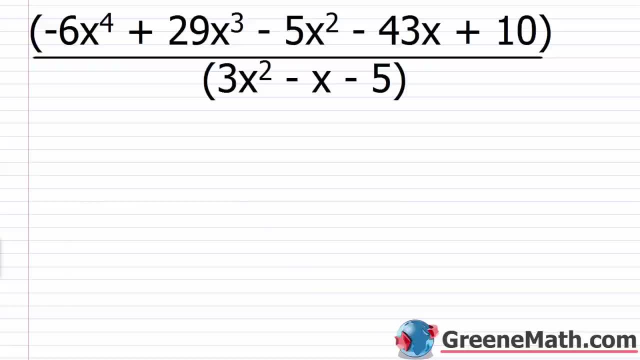 16, I would get exactly that. All right, let's take a look at one more where there's not a remainder, And then I'm going to go through what happens when there is a remainder. We'll just look at an example of that. So we have negative 6x to the fourth power, plus 29x cubed, minus 5x squared. 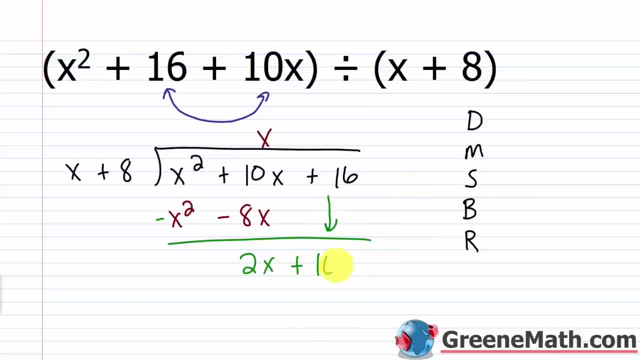 Now we're going to bring down to plus 16, and then we're going to repeat. So we go back up to the top. So we're going to go leading term into leading term. So what is 2x over x? Well, the x's would 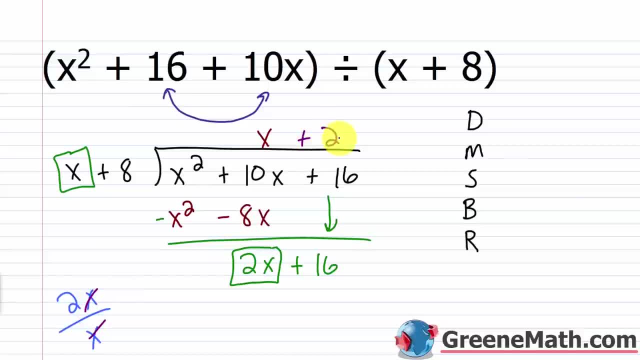 cancel, and I would just have a 2, so plus 2. Again, multiply. 2 times x is 2x. 2 times 8 is plus 16. So we could see we wouldn't have a remainder here, right? Anything minus itself is 0. 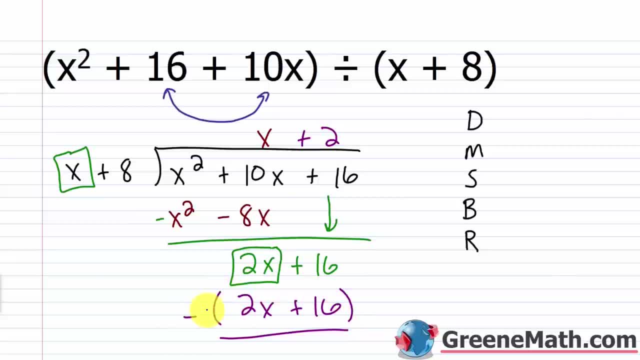 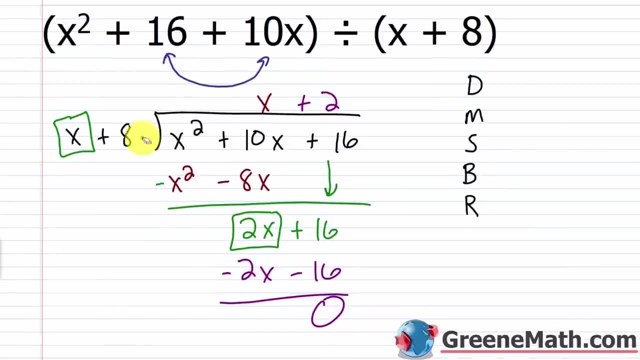 But again, if we were to do it again, we would have to do it again. So we're going to do it again. the sake of completeness we're going to subtract this away so i'm going to change the sign of each term this will be minus and that'll be minus and i can erase this 2x minus 2x is 0 16 minus 16 is 0. so again there's no remainder so our answer here is x plus 2. so x plus 2 and it's very very easy to check so again if i wanted to take the quotient x plus 2 and multiply that by the divisor x plus 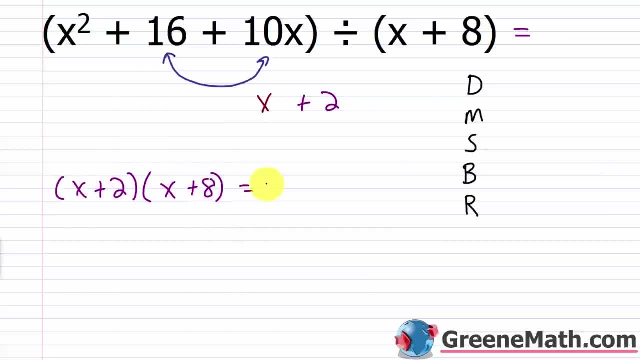 8 i should get my dividend back x times x is x squared x times 8 is plus 8x 2 times x is plus 2x 2 times 8 is plus 16. so if i combine like terms i get x squared plus 10x plus 16 which is exactly this just looks a little different because this is not in standard form and this is right but if 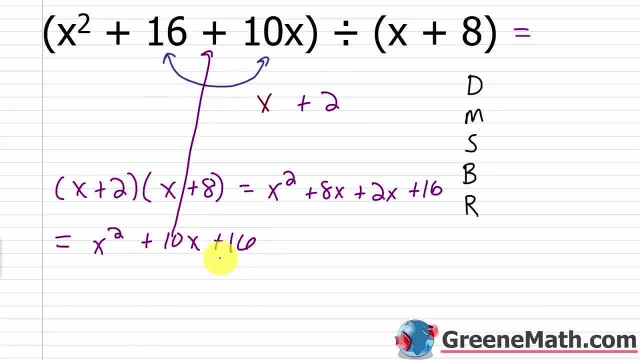 i flip the position here of the 10x and the 16 i would get exactly that all right let's take a look at one more where there's not a remainder 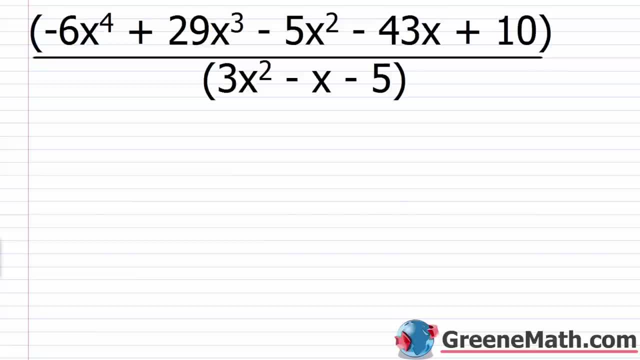 and then i'm going to go through what happens when there is a remainder we'll just look at one example of that so we have negative 6x to the fourth power plus 29 x cubed minus 5x squared minus 43x plus 10 and then i'm dividing this by 3x squared minus x minus 5. all right so let's go ahead and set this guy up so this is my dividend so that's going to go under the house so negative 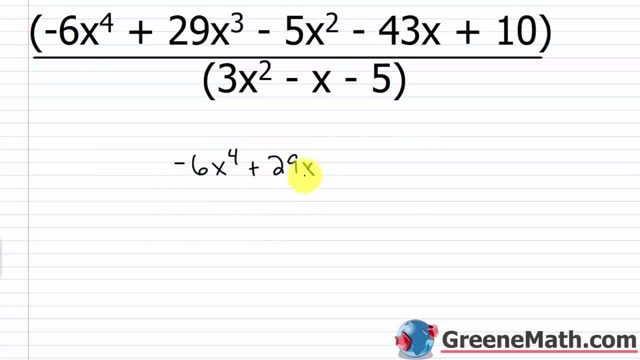 6x to the fourth power plus 29 x cubed 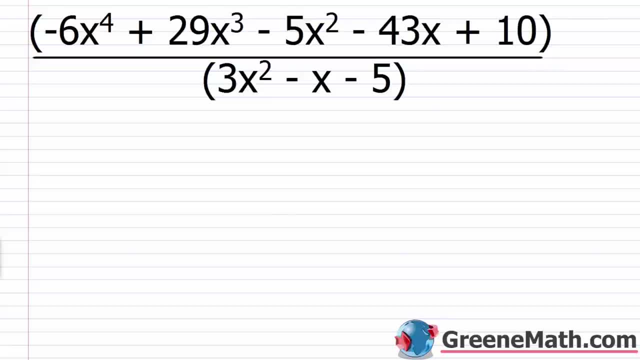 minus 43x plus 10.. And then I'm dividing this by 3x squared minus x minus 5.. All right, so let's go ahead and set this guy up. So this is my dividend. So that's going to go under the house. 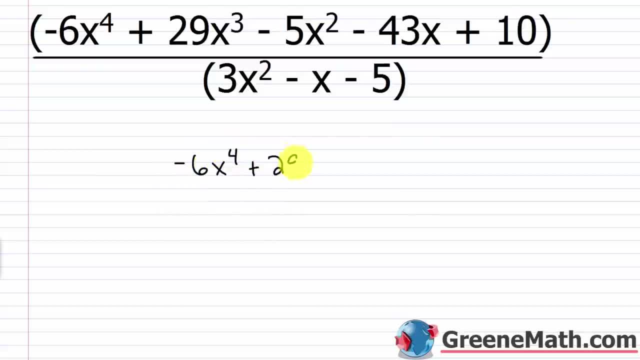 Negative: 6x to the fourth, power plus 29x cubed minus 5x squared minus 43x plus 10x. Again, that goes under the house And then off to the left, we have 3x squared minus x minus 5.. 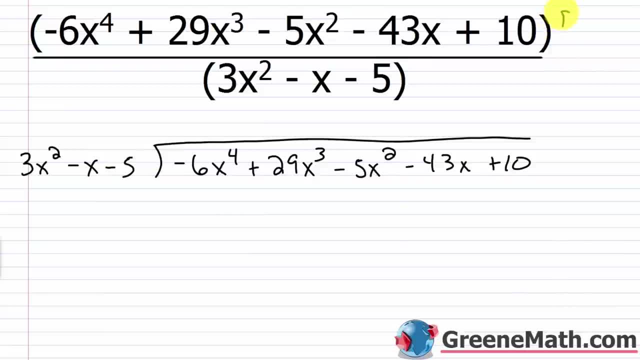 So again, let me write the steps up here so we don't forget. So we have divide, we have multiply, we have subtract, we have bring down, and then we have repeat or remainder right, Dad, mom, sister, brother, rover. So we start out with the first step, leading term. 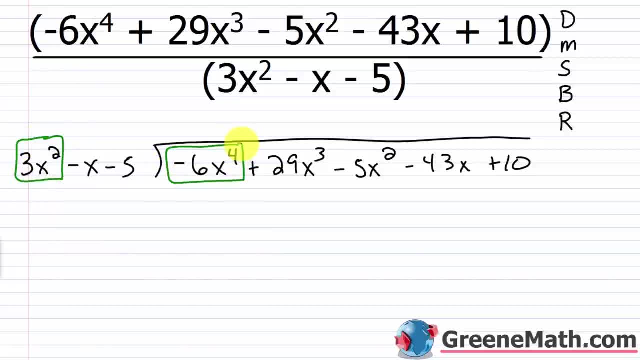 into leading term. 3x squared into negative 6x to the fourth power, So negative 6x to the fourth power over 3x squared. So this negative 6 will cancel with 3 and give me negative 2.. X to the fourth will cancel with. 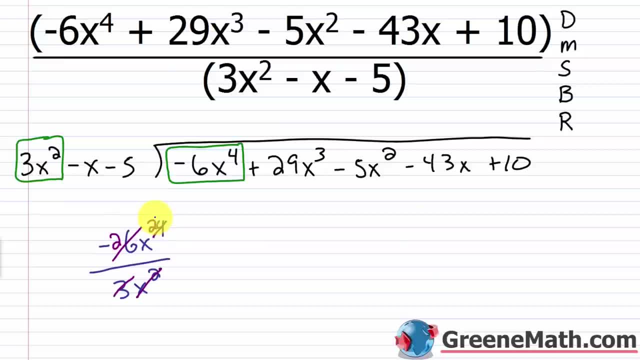 x squared and give me x squared, So negative, 2x squared is the answer. Where am I going to write that? Am I going to write it here, over the x fourth spot? No, Am I going to write it here over the x cubed spot? No, I'm going to write it over the x squared spot, because that's where it goes. 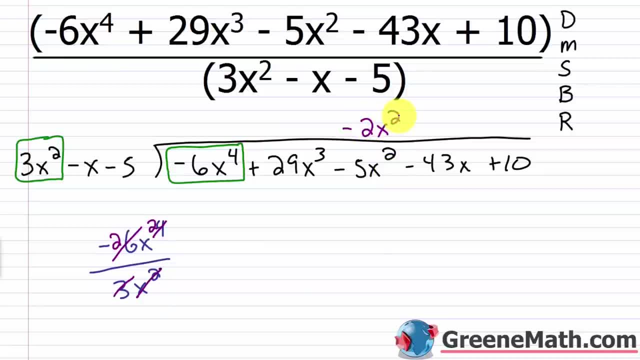 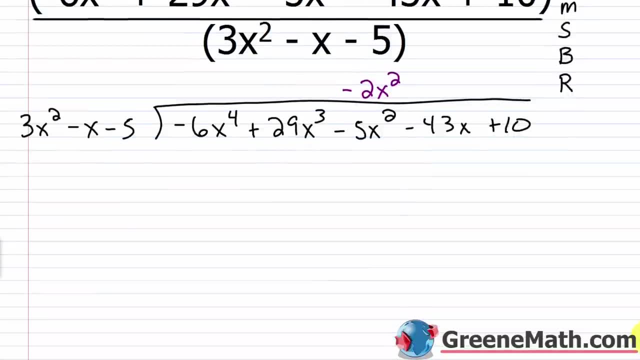 So negative 2x squared. All right, now I'm going to multiply. That's my next step. Let me erase this stuff And let me scroll down a little bit, And I realize it's going to take this guy off the screen. 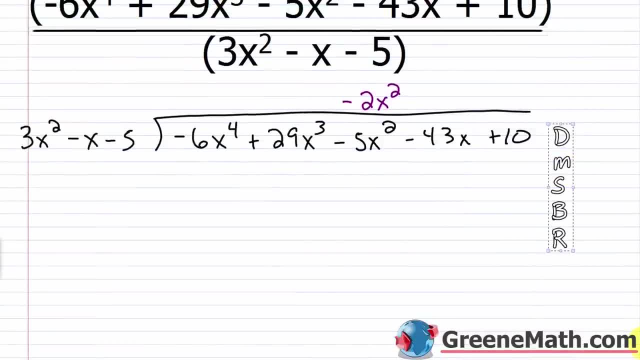 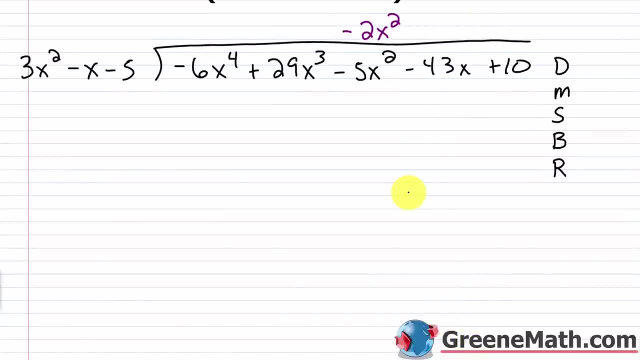 So let me kind of drag this down right there And let me scroll down a little bit. There we go. Okay, so now again we're multiplying Negative 2x squared times 3x squared is going to be negative 6x to the fourth power. 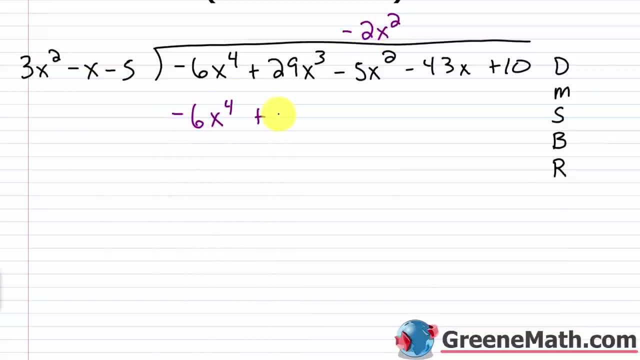 Negative 2x squared times negative. x is positive: 2x cubed. Negative 2x squared times negative. 5 is going to be positive, 10x squared. Now I am subtracting this thing away. Remember. usually what I do is I put parentheses around here, put a minus out in front. 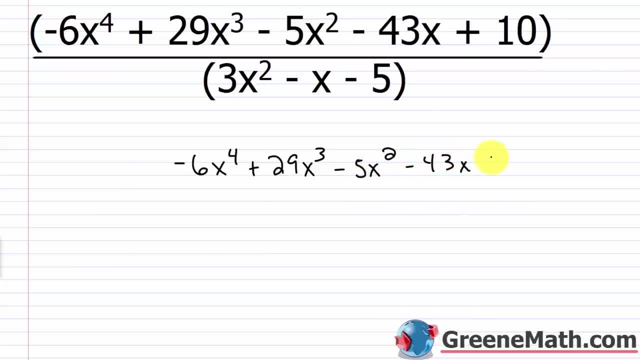 minus 5x squared minus 43x plus 10. again that goes under the house and then off to the left we have 3x squared minus x minus 5. so again let me write the steps up here so we don't forget so we have divide we have multiply we have subtract we have bring down and then we have repeat or remainder right dad mom sister brother rover so we start out with the first step leading term 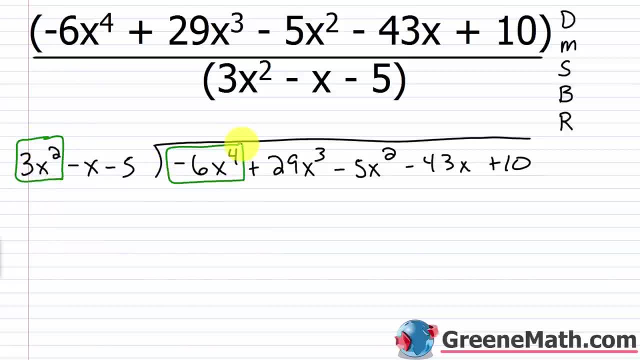 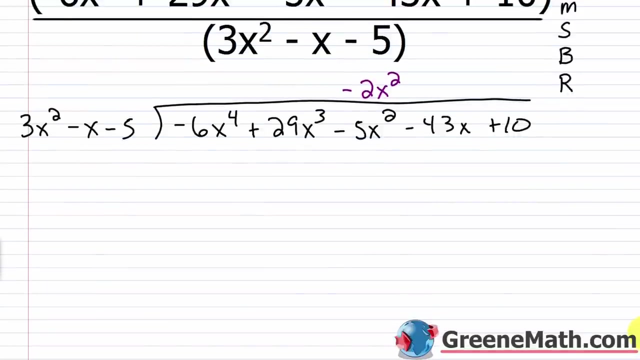 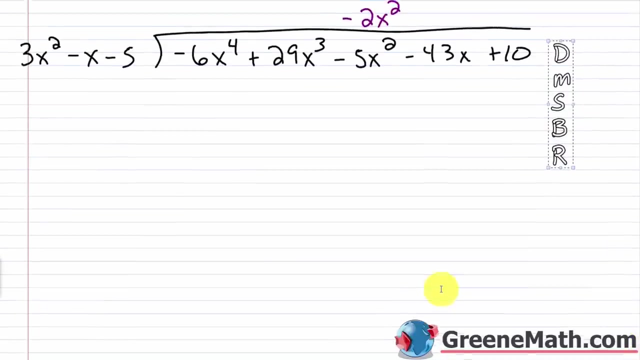 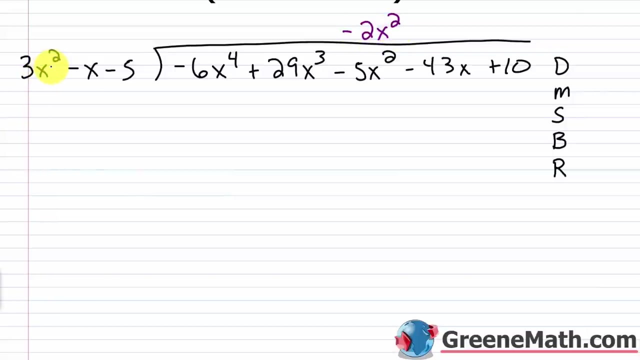 into leading term so 3x squared into negative 6x to the fourth power so negative 6x to the fourth power over 3x squared so this negative 6 will cancel with 3 and give me negative 2 x to the fourth will cancel with x squared give me x squared so negative 2x squared is the answer where am i going to write that am i going to write it here over the x fourth spot no am i going to write it here over the x cube spot no i'm going to write it over the x squared spot because that's where it goes so negative 2x squared all right now i'm going to multiply that's my next step let me erase this stuff and let me scroll down a little bit and i realize it's going to take this guy off the screen so let me kind of drag this down right there and let me scroll down a little bit there we go okay so now again we're multiplying negative 2x squared times three x squared is going to be negative 6x to the fourth power 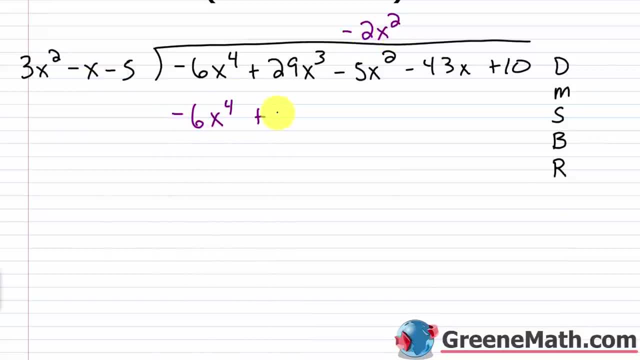 negative two x squared times negative x is positive two x cubed negative two x squared times negative five is gonna be positive 10 x squared now i am subtracting this thing away remember usually what i do is i put parentheses around here put a minus out in front you don't need to do that if you just change the sign a of everything. So this is minus, it's going to become plus. This is plus, it's going to become minus. This is plus, it's going to become minus. Now I can just add. Negative 6x to the fourth power plus 6x to the fourth power is 0. 29x cubed minus 2x cubed is 27x cubed. Negative 5x squared minus 10x squared is minus 15x squared. And then I want to bring down. So bring down the negative 43x. And then we're going to repeat. So I'm going to go leading term into leading term. 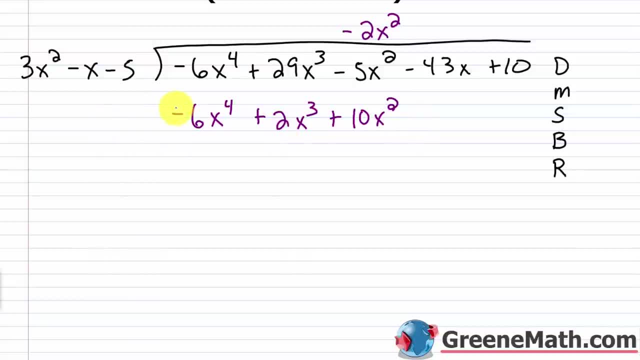 You don't need to do that if you just change the sign of everything. So this is minus, it's going to become plus. This is plus, it's going to become minus. This is plus, it's going to become minus. Now I can just 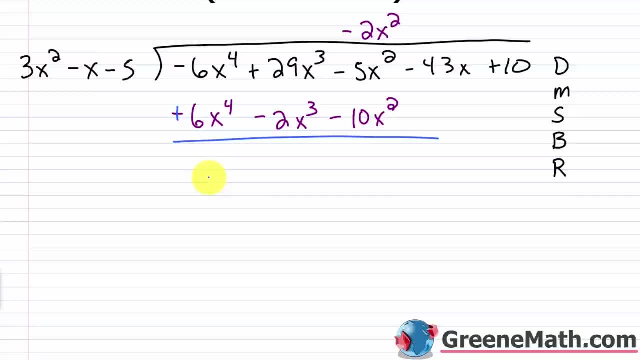 Add negative 6x to the fourth power. plus 6x to the fourth power is 0.. 29x cubed minus 2x cubed is 27x cubed. Negative: 5x squared minus 10x squared is minus 15x squared. 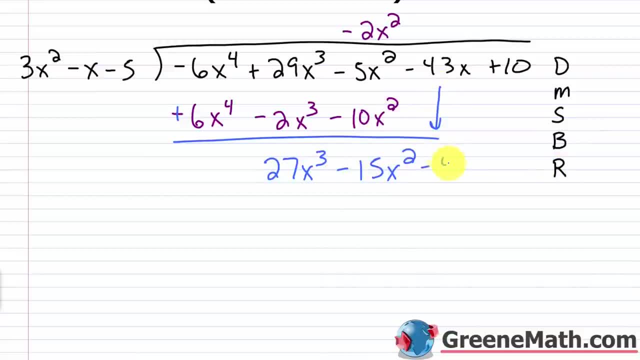 And then I want to bring down. So bring down the negative 43x, And then we're going to repeat. So I'm going to go leading term into leading term. So what is 27x cubed over 3x squared? 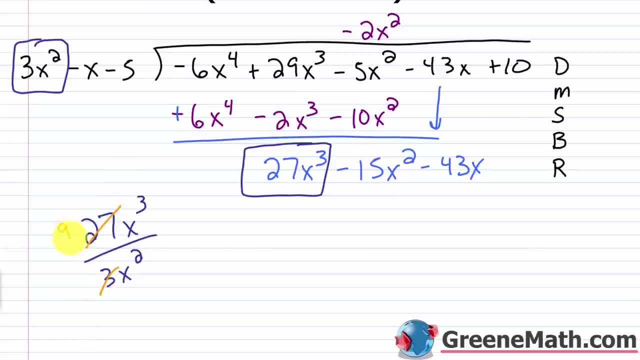 Well, I know 27 divided by 3 is 9.. X cubed over x squared would be x to the first power. So I'm going to put plus 9x, Okay, And then I'm going to multiply. Let's erase this. 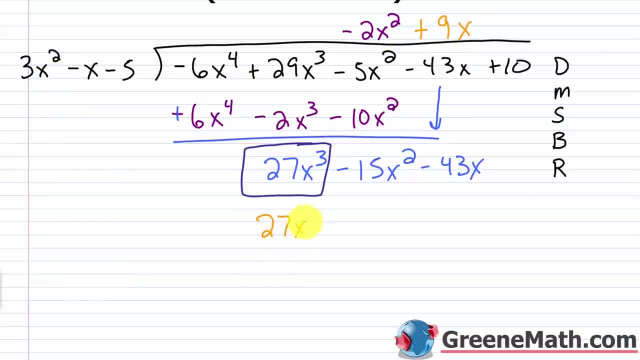 So 9x times 3x squared is 27x cubed. 9x times negative, x is negative. 9x squared, 9x times negative, 5 is minus 45x squared. Again, I am subtracting this away. 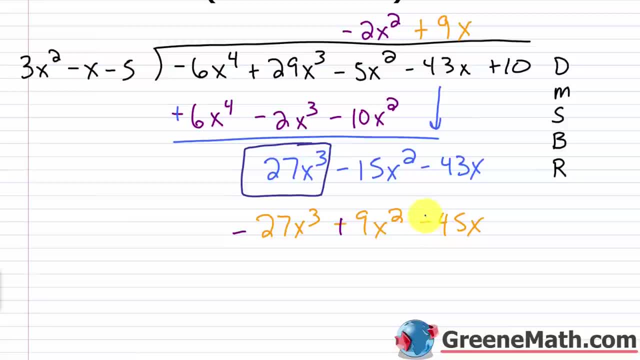 So just change the sign of everything. So this will be minus, plus, plus. Now I can just add 27x cubed. minus 27x cubed is 0.. Negative: 15x squared plus 9x squared is negative: 6x squared. 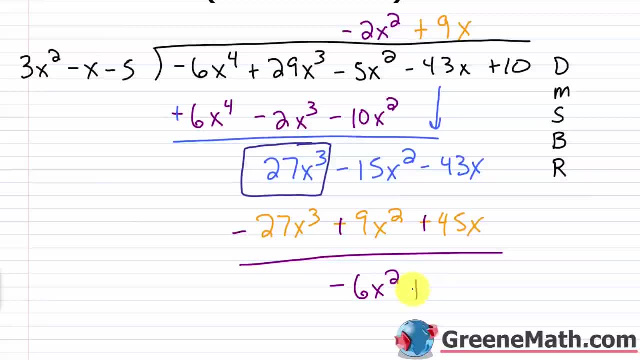 Negative: 43x plus 45x is positive 2x. Now we're going to bring down, Bring down this plus 10.. Then we want to repeat, So I'm going to again go leading term, Leading term, into leading term. 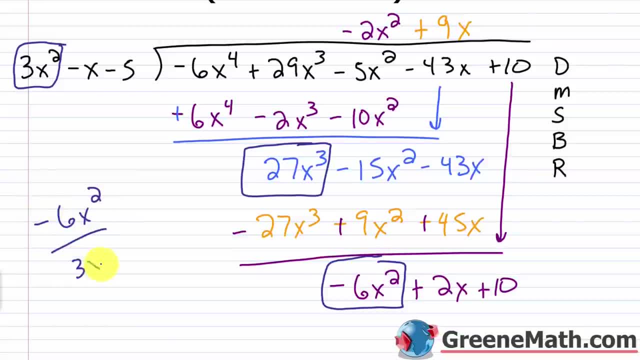 So what is negative? 6x squared over 3x squared. Well, x squared over x squared is going to cancel Negative. 6 over 3 is negative 2.. So this will just be minus 2 here, And then one last time I'm going to multiply. 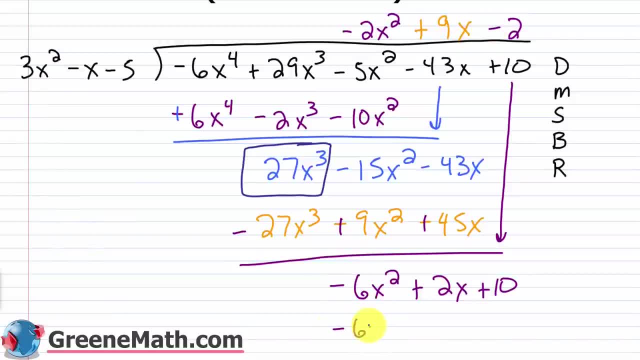 So negative 2 times 3x squared is negative. 6x squared Negative 2 times negative: x is plus 2x. Negative 2 times negative: 5 is plus 10.. So you can see it's the same thing minus itself. 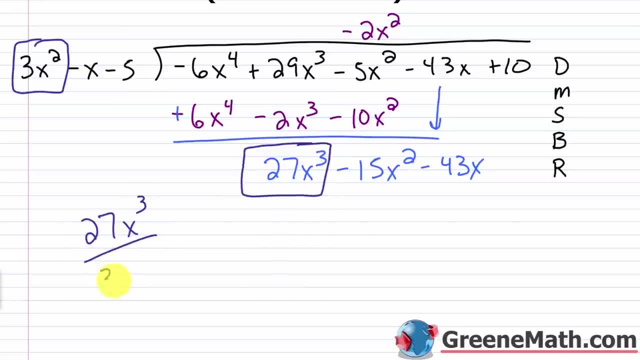 So what is 27x cubed over 3x squared? Well, I know 27 divided by 3 is 9. x cubed over x squared would be x to the first power. So I'm going to put plus 9x. Okay. And then I'm going to multiply. Let's erase this. 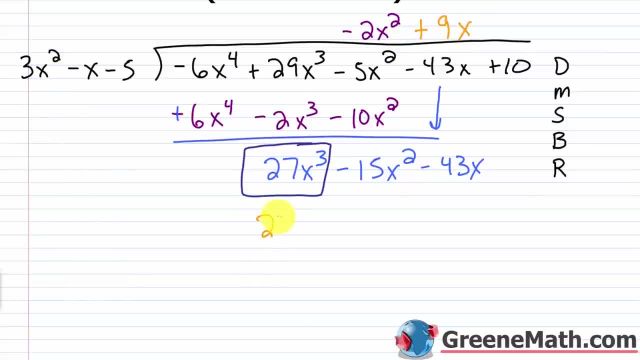 So 9x times 3x squared is 27x cubed. 9x times negative x is negative 9x squared. 9x times negative 5 is minus 45x. Again, I am subtracting this away. So just change the sign of everything. So this will be minus plus plus. Now I can just add. 27x cubed minus 27x cubed is 0. Negative 15x squared plus 9x squared is negative 6x squared. 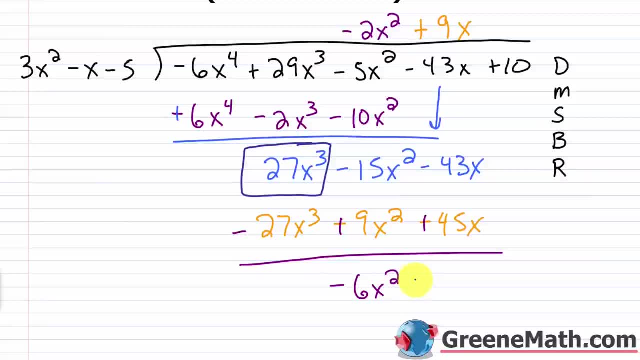 Negative 43x plus 45x is positive 2x. Now we're going to bring down. Bring down this plus 10. 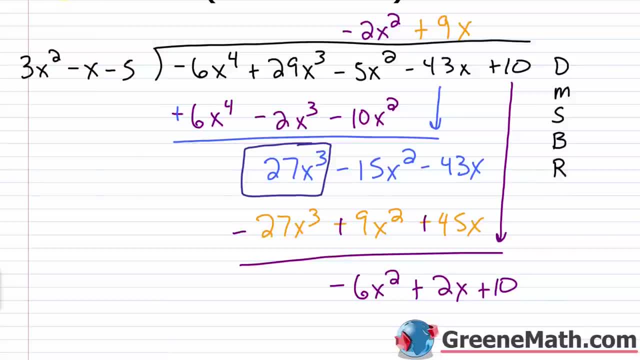 Then we want to repeat. So I'm going to again go leading term, leading term into leading term. 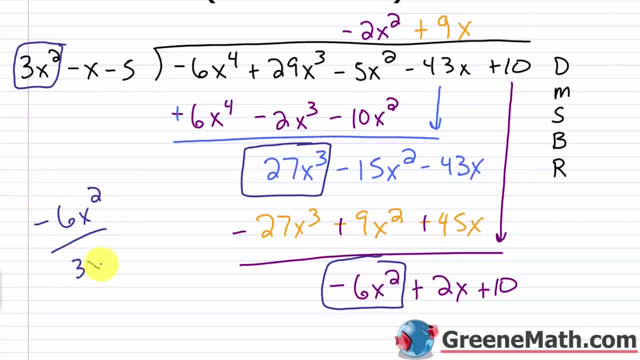 So what is negative 6x squared over 3x squared? Well, x squared over x squared is going to cancel. Negative 6 over 3 is negative 2. So this will just be minus 2x squared over 3x squared. So I'm going to leave negative 2 here. And then one last time I'm going to multiply. So negative 2 times 3x squared is negative 6x squared. Negative 2 times negative x is plus 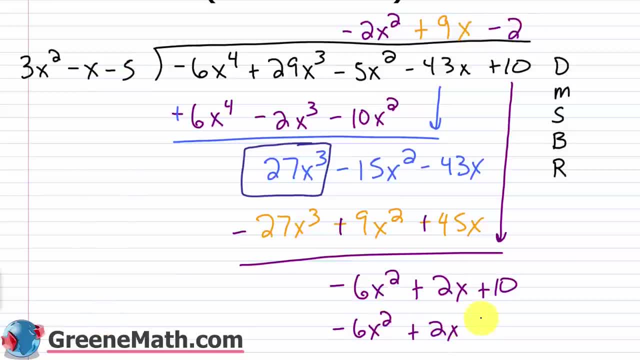 2x. Negative 2 times negative 5 is plus 10. So you can see it's the same thing minus itself. That would be 0. But again, to kind of make this complete, if I'm subtracting this away, I'm going to change every sign. So this will be plus. This will be minus. This will be 2x squared. This will be minus. And then if we add it here, 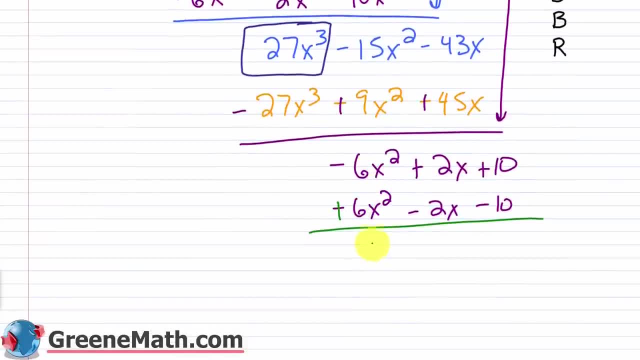 negative 6x squared plus 6x squared is 0. 2x minus 2x is 0. 10 minus 10 is 0. So that's 0. 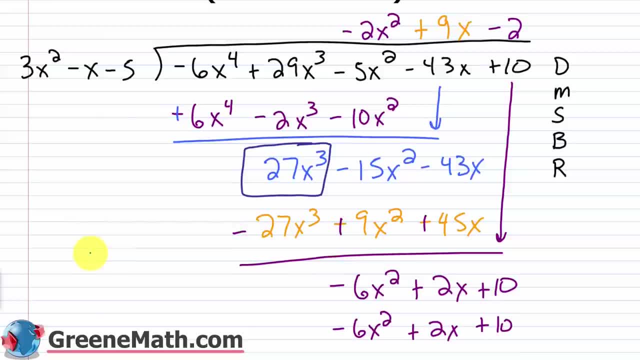 That would be 0. But again, to kind of make this complete, if I'm subtracting this away, I'm going to change every sign. So this will be plus, This will be minus, This will be minus. And then, if we add it here, 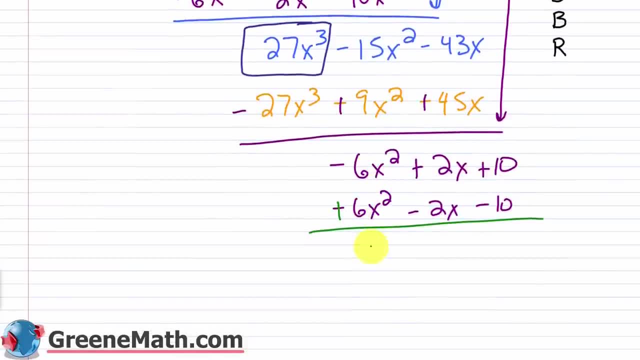 negative: 6x squared plus 6x squared is 0.. 2x minus 2x is 0.. 10 minus 10 is 0.. So that's 0.. So there is no remainder, So let me erase everything. 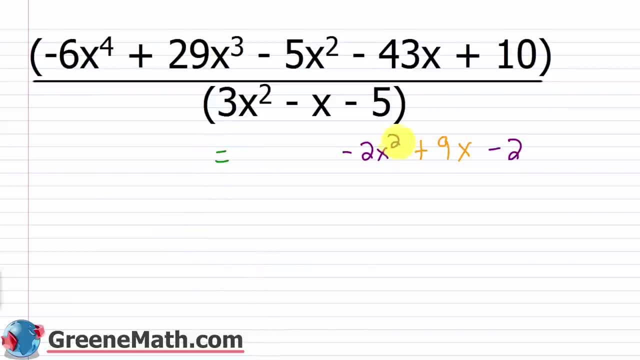 So this is equal to that. And so again, if we want to check, you're going to take this guy. multiply by this guy. So negative 2x squared plus 9x minus 2 would be multiplied by 3x squared minus x minus 5.. 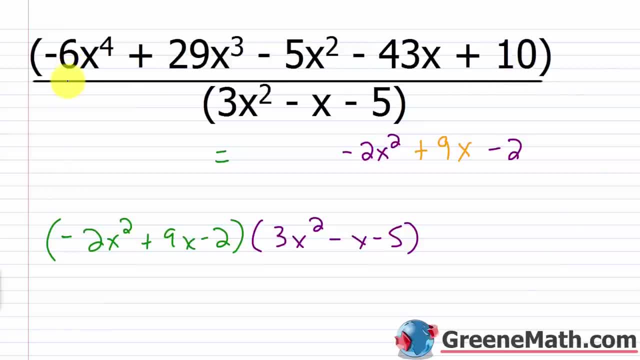 And I should get this long thing up here. on the top right, The negative 6x to the fourth power plus 29x cubed, minus 5x squared, minus 43x plus 10.. So let's see if we do in fact get that. 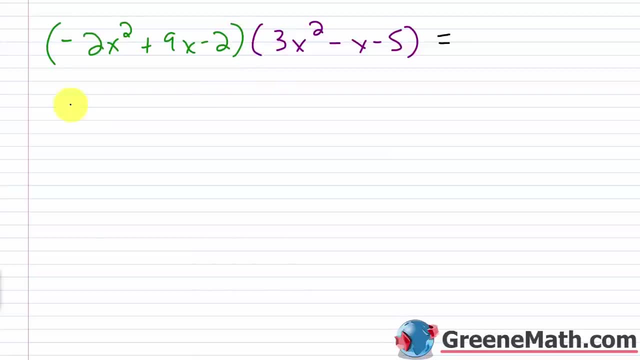 Okay, so let's begin. We have negative 2x squared times 3x squared, That's negative 6x to the fourth power. I have negative 2x squared times negative x, That's positive 2x cubed. 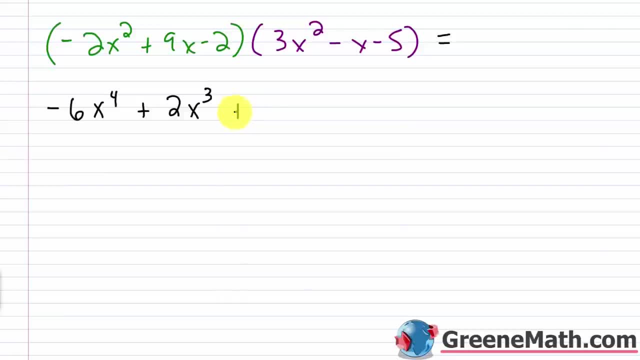 I have negative 2x squared times negative 5. That's positive 10x squared. Then I have 9x times 3x squared, That's plus 27x cubed. I have 9x times negative x, That's minus 9x squared. 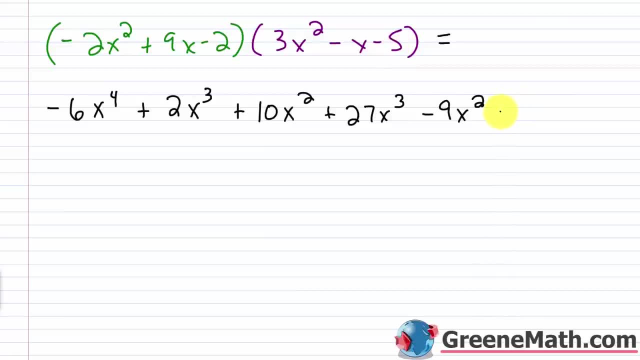 And then I have 9x, 9x times negative, 5. That's minus 45x. Then I have negative 2 times 3x, That's minus 6x. squared Negative 2 times negative: x, That's plus 2x. 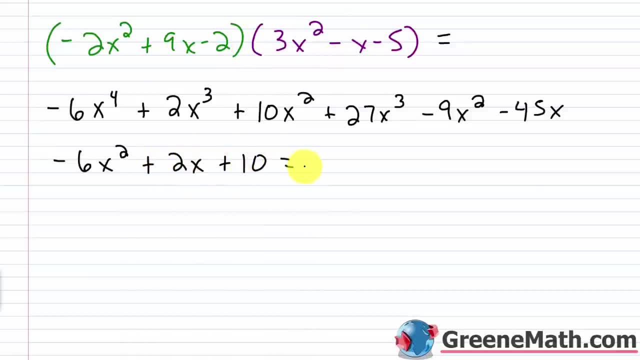 And then negative 2 times negative, 5 is plus 10.. All right, so if I combine like terms here, I'm going to get negative 6x to the fourth power. I have a cubed here and here. So 2 plus 27 is 29.. 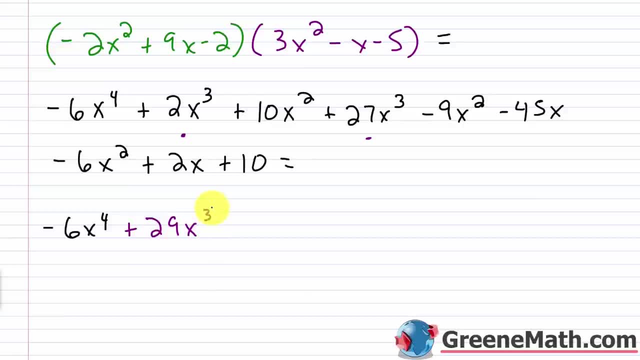 So plus 29x cubed, Then I have 10x squared, negative 9x squared and negative 6x squared. So 10 minus 9 is 1.. 1 minus 6 is negative 5. So this would be minus 5x squared. 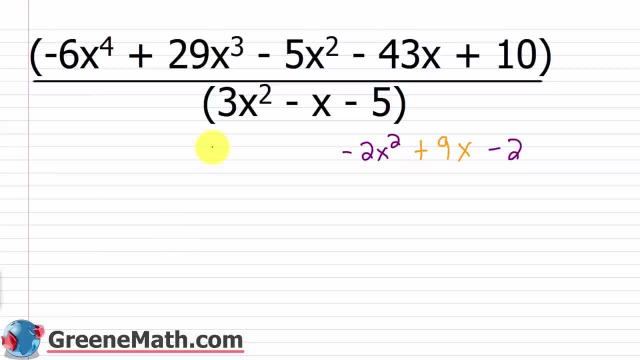 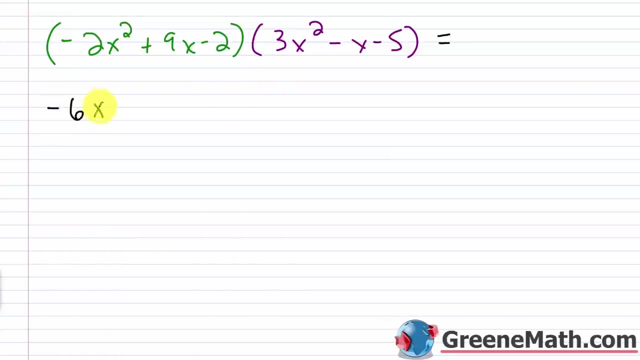 So there is no remainder. So let me erase everything. So this is equal to that. And so again, if we want to check, you're going to take this guy, multiply by this guy. So negative 2x squared plus 9x minus 2 would be multiplied by 3x squared, minus x minus 5. And I should get this long thing up here on the top, right? The negative 6x to the fourth power plus 29x cubed minus 5x squared minus 43x plus 10. So let's see if we do in fact get that. Okay, so let's begin. We have negative 2x squared times 3x squared. That's negative 6x to the fourth power. I have negative 2x squared times negative x. That's positive 2x cubed. I have negative 2x squared times. Negative 5. That's positive 10x squared. Then I have 9x times 3x squared. That's plus 27x cubed. I have 9x times negative x. That's minus 9x squared. And then I have 9x times negative 5. That's minus 45x. Then I have negative 2 times 3x. That's minus 6x squared. Negative 2 times negative x. That's plus 2x. And then negative 2 times negative 5 is plus 10. All right, so if I combine like terms here, I'm going to get negative 6x to the fourth power. I have a cubed here and here. So 2 plus 27 is 29. 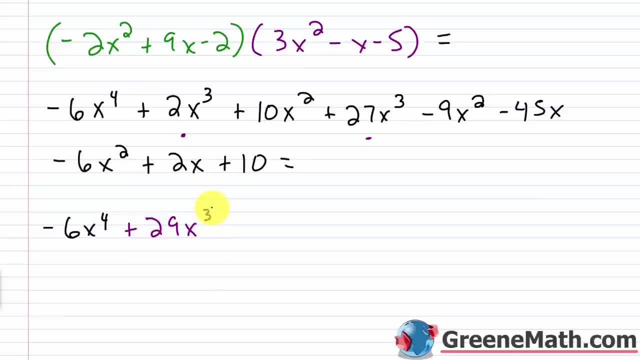 So plus 29x cubed. Then I have 10x squared, negative 9x squared, and negative 6x squared. So 10 minus 9 is 1. 1 minus 6 is negative 5. So this would be minus 5x squared. Then I'm looking at 5x and 2x. Negative 45 plus 2 is negative 43. So minus 43x. And then lastly, plus 10. This is 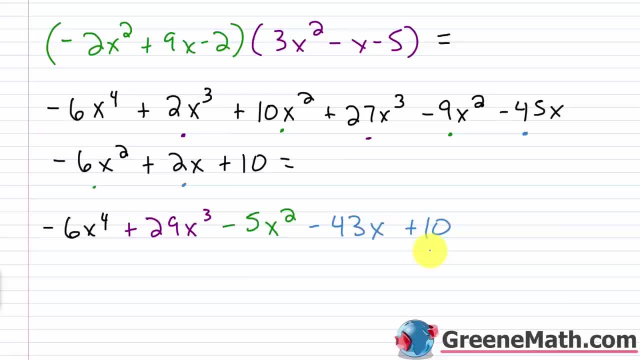 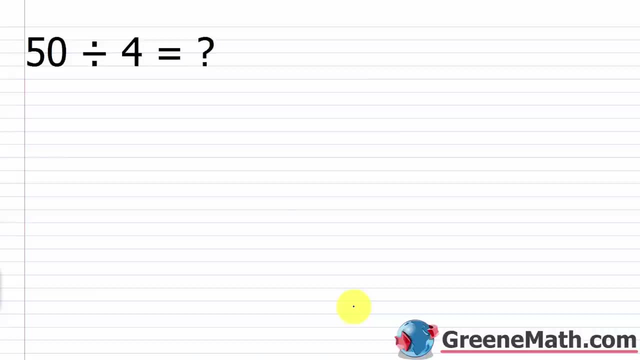 exactly what we started out with as our dividend. Negative 6x to the fourth power plus 29x cubed minus 5x squared minus 43x plus 10. All right, so now let's talk a little bit about what to do when 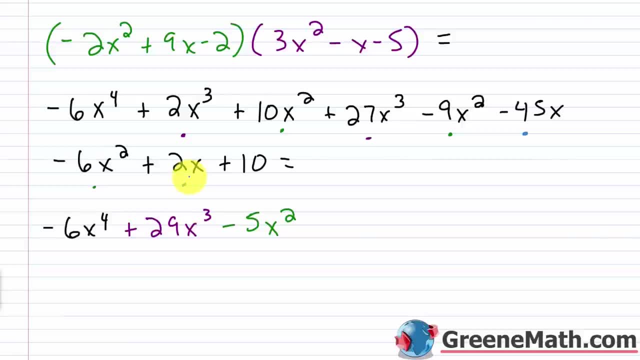 Then I'm looking at negative 45x and 2x. Negative 45 plus 2 is negative 43.. So minus 43x, And then lastly, plus 10.. This is exactly what we started out with as our dividend. 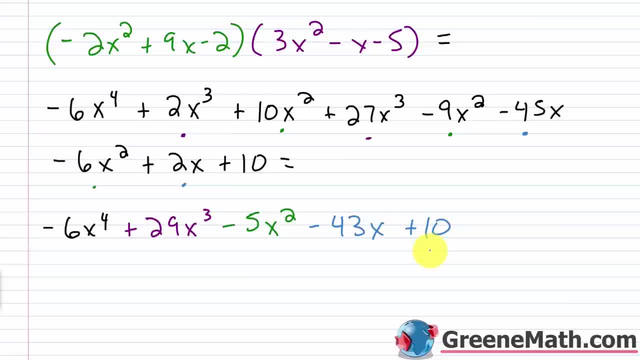 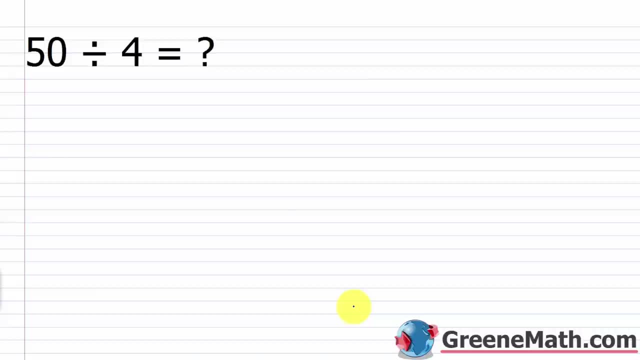 Negative 6x to the fourth, power plus 29x, cubed Minus 5x, squared minus 43x plus 10.. All right, so now let's talk a little bit about what to do when your division problem with polynomials has a remainder. 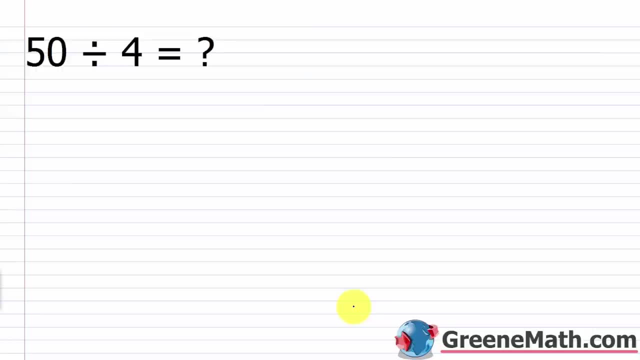 So I want to go back to a problem that we would have encountered in grammar school. So something like 50 divided by 4.. 50 is not divisible by 4 because when the division is concluded you have a remainder right. So we could say that 50 divided by 4.. 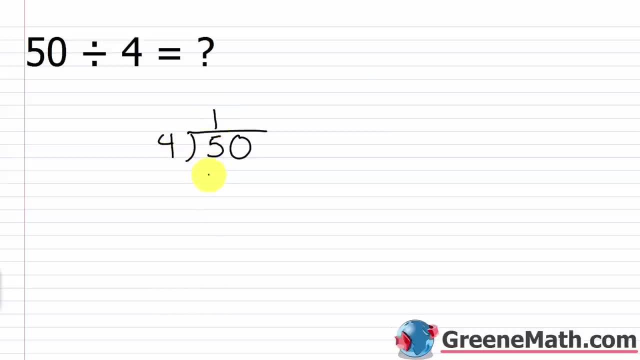 We'd start with 4.. We'd start with 4.. We'd start out with saying: 4 goes into 5 once. 1 times 4 is 4.. Subtracting, you get 1.. Bring down the 0.. 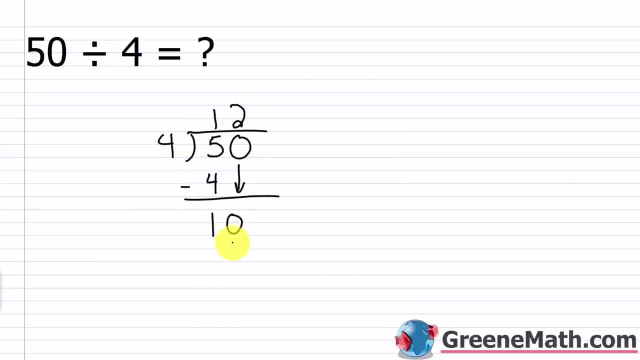 4 goes into 10. twice 2 times 4 is 8.. Subtracting you get 2.. So this 2 is known as a remainder right. So remember, kind of in grammar school we wrote this as 12R2, right? 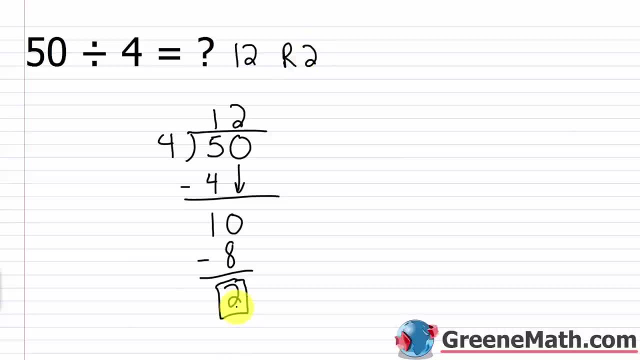 That was the remainder, That was the leftover amount. So in other words, to kind of break this down completely, if I took 50 and I split it up, I could make 12 groups right. 12 times 4 is 48.. 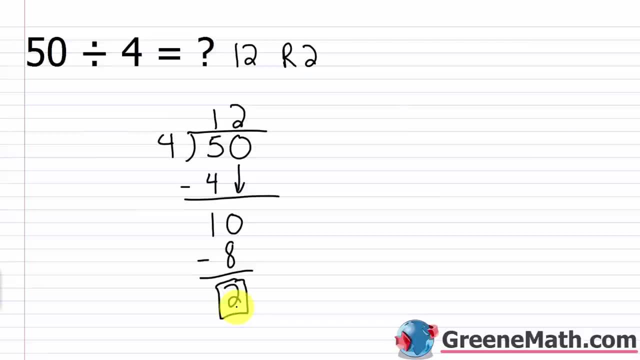 And then I would have 2 left over, right? So 48 plus 2 would get you back to 50. The remainder is kind of what I have left over. I don't. I don't have enough to make another group of 4.. 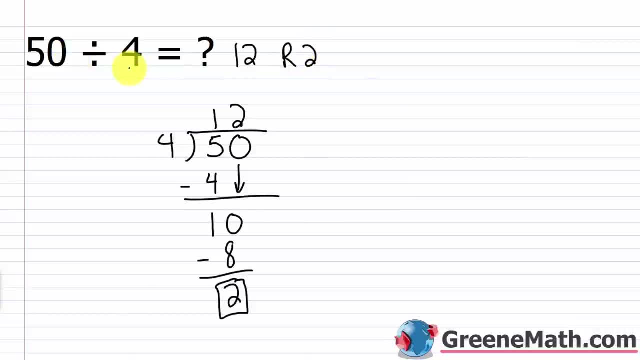 So that's how that comes about. But we learned a couple of different things that we could do. The first thing we kind of did was we put a decimal point here, We're bringing that up here, We put a 0 and we continue our division. 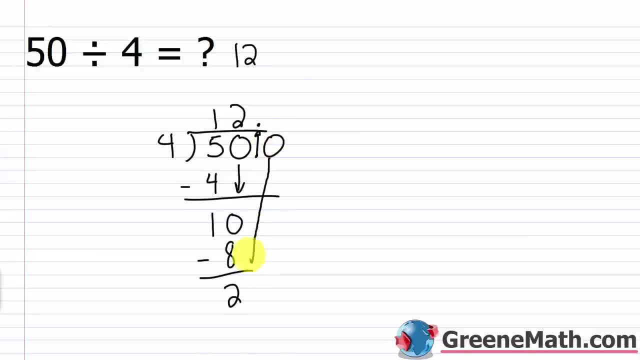 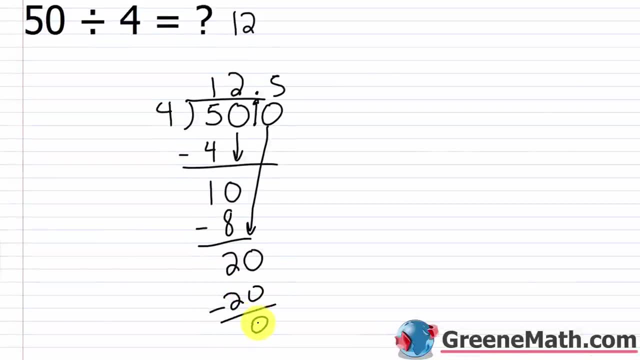 4 goes into 25 times. 5 times 4 is 20.. Subtracting you get 0. So that's what we're going to do: Subtracting you get 0.. So now I know the answer is 12.5 in decimal form. 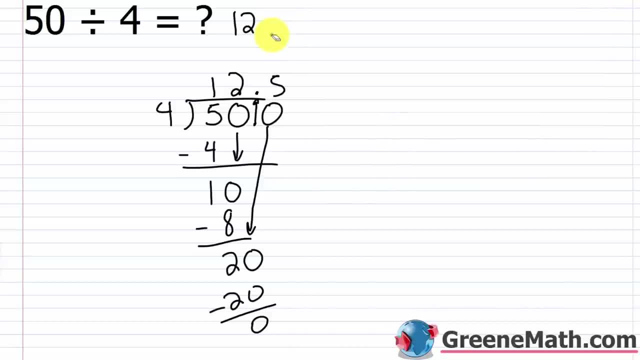 But that's not really going to help us with polynomial division. The other way we could have written this. think about the .5 there. we could have gone back to this. let me erase all this and said that this remainder 2,. 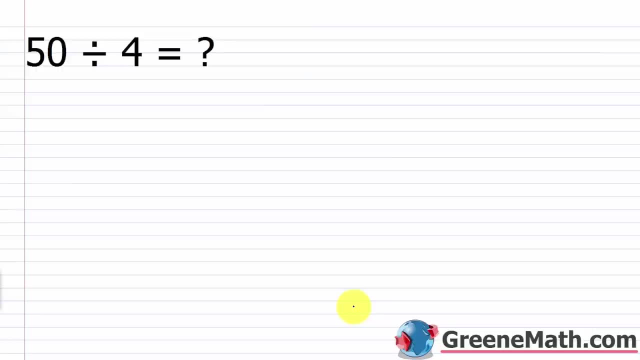 your division problem with polynomials has a remainder. So I want to go back to a problem that we would have encountered in grammar school. So something like 50, divided by 4. 50 is not divisible by 4 because when the division is concluded, you have a remainder, right? So we could say that 50 divided by 4, we'd start out with saying 4 goes in a 5 once. 1 times 4 is 4. Subtracting, you get 1. Bring down the 0. 4 goes in a 10 twice. 2 times 4 is 8. Subtracting, you get 2. So this 2 is known as a remainder, 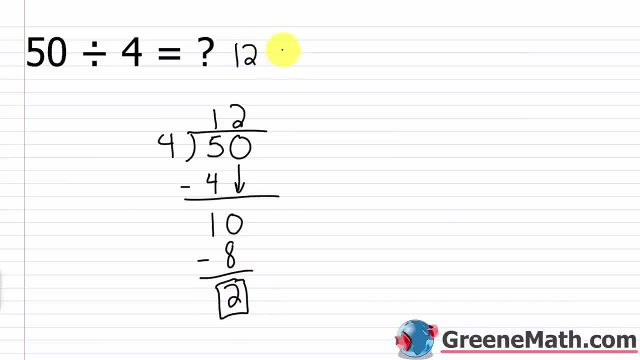 right? So remember kind of in grammar school, we wrote this as 12R2, right? That was the remainder. 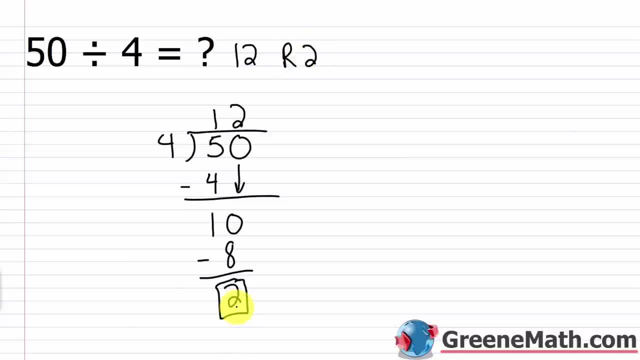 That was the leftover amount. So in other words, to kind of break this down completely, if I took 50 and I split it up into equal groups of four, I could make 12 groups, right? 12 times 4 is 48. And then I would have 2 left over, right? So 48 plus 2 would get you back to 50. The remainder is kind of what I have left over. I don't have enough to make another group of 4. So that's how that could work. 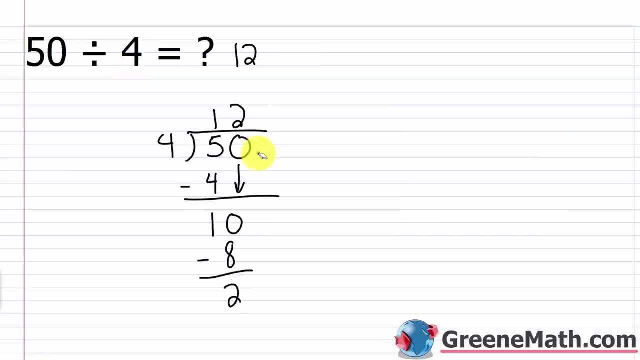 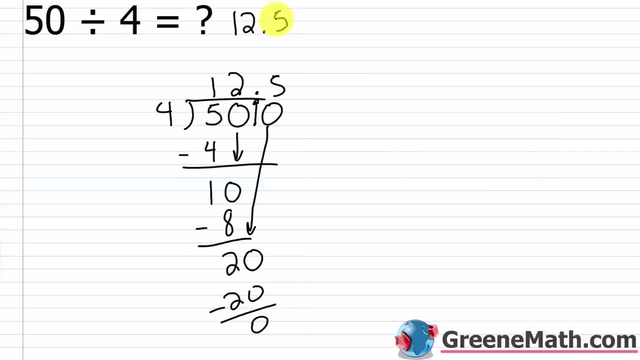 comes about but we learned a couple of different things that we could do the first thing we kind of did was we put a decimal point here we're bringing that up here we put a zero and we continue our division four goes into 25 times five times four is 20 subtracting you get zero so now i know the answer is 12.5 in decimal form but that's not really going to help us with polynomial division the other way we could have written this think about the 0.5 there we could have gone back to this let me erase all this and say that this remainder two we could say plus i have two that's divided by four or i have 12 plus one half right two over four is one half and we know that 12 plus one half or 12 plus in decimal form 0.5 is 12.5 that's exactly what we got when we continued the division so it's legal to write it as 12 plus one half or as a mixed number right 12 and one half like that this is how we're going to write our answers 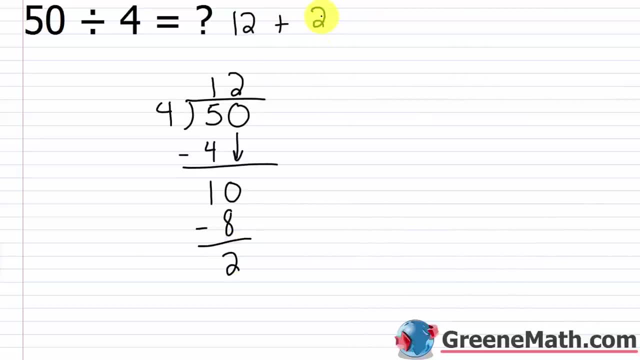 we could say: plus I have 2, that's divided by 4.. Or I have 12 plus 1 half. Right, 2 over 4 is 1 half, And we know that 12 plus 1 half or 12 plus in decimal form. 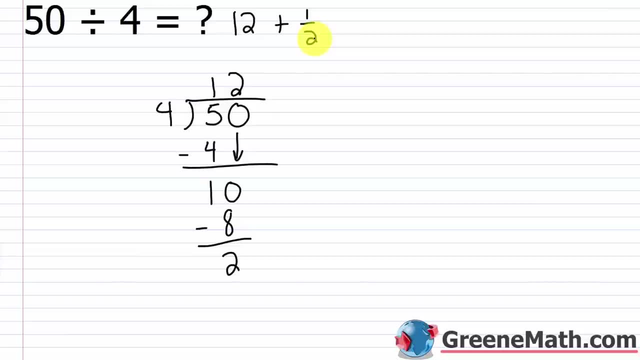 .5 is 12.5.. That's exactly what we got when we continued the division, So it's legal to write it as 12 plus 1 half or as a mixed number. write 12 and 1 half like that. 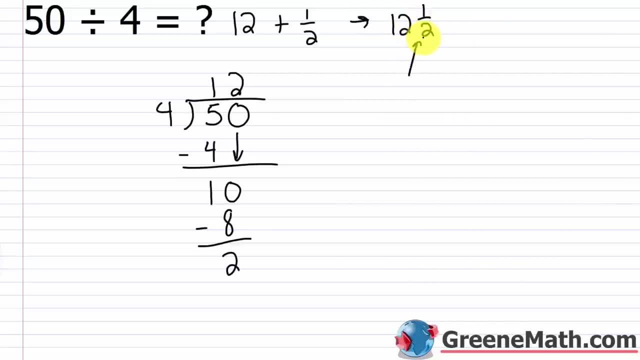 This is how we're going to write our answers when we're dividing with polynomials. We're going to write it in that format. You'll have your quotient plus, you'll take the remainder and put it over the divisor. Now, this is very, very important. 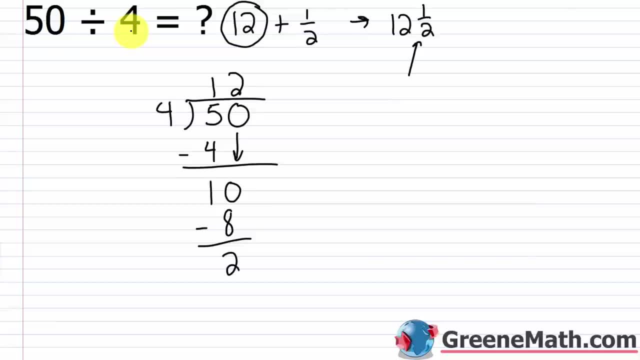 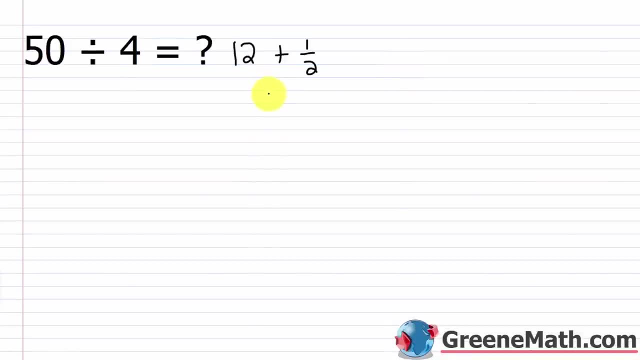 When you check your result, it's a little bit more complex. Let me erase this real quick. If I was to check the answer here, what would I do? Well, I could multiply this whole thing right here in this format: times 4.. So I could say 4 times. 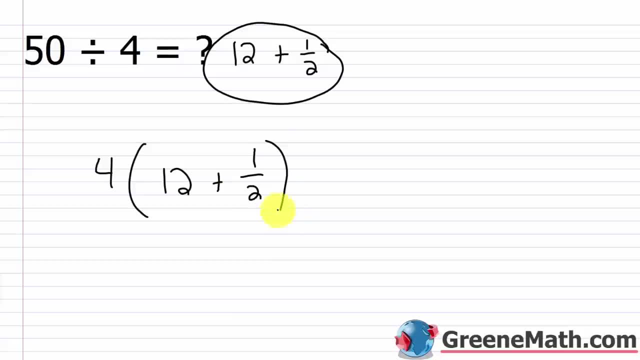 12 plus 1 half. 4 times 12 is 48.. Plus 4 times 1 half is 2.. And that would get me back to 50. So I can do it that way. Another way that I could do this: 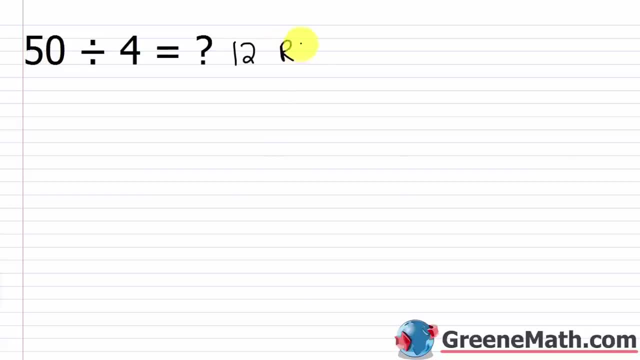 I could go back to kind of 12 R2, and I could say, okay, 12,. the quotient times 4 is 48, add the remainder back in, I get to 50. So those are kind of two different ways that you can look at that. 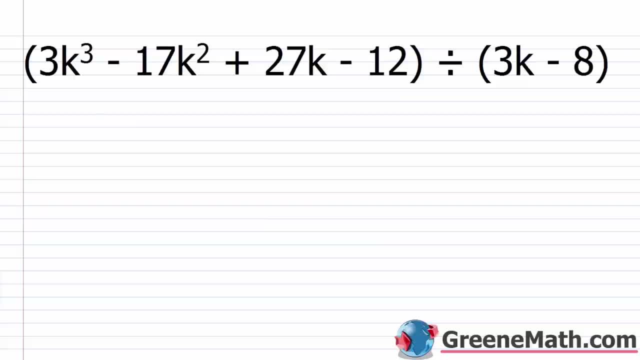 Alright, so let's take a look at our problem. So we have 3k cubed minus 17k, squared plus 27k minus 12, and I'm dividing by 3k minus 8.. So again, this guy goes under the house. so 3k. 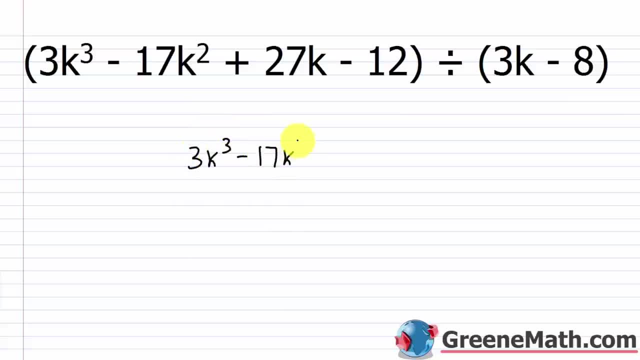 cubed minus 17k, squared plus 27k minus 12, and we're going to divide this by again, 3k minus 8.. So I can keep writing this off to the side. So division, multiplication subtract, bring down. 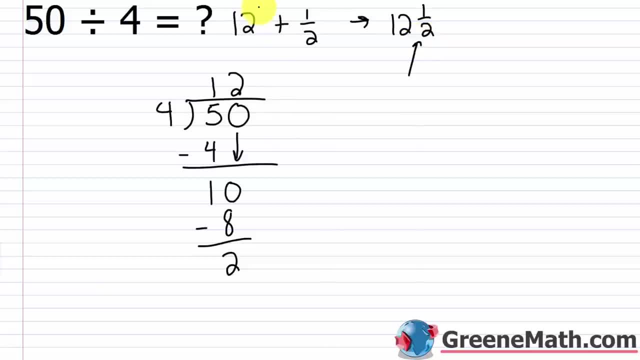 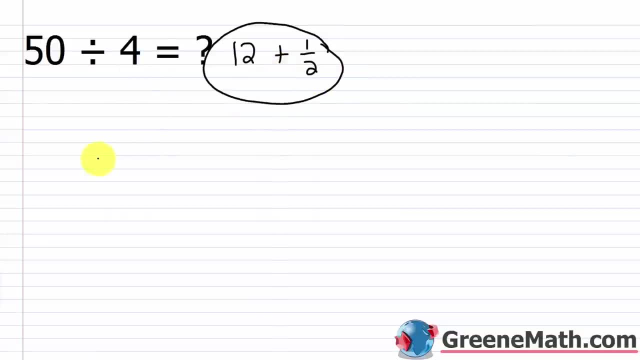 multiply the answer by the divisor and i could multiply this whole thing right here in this format times four so i could say four times 12 plus one half four times 12 is 48 plus four times one half is two and that would get me back to 50 so i can do it that way another way that i could do this i could go back to kind of 12 r2 and i could say okay 12 the quotient times four is 48 add the remainder back in i get to 50 right so those kind of two different ways that you can 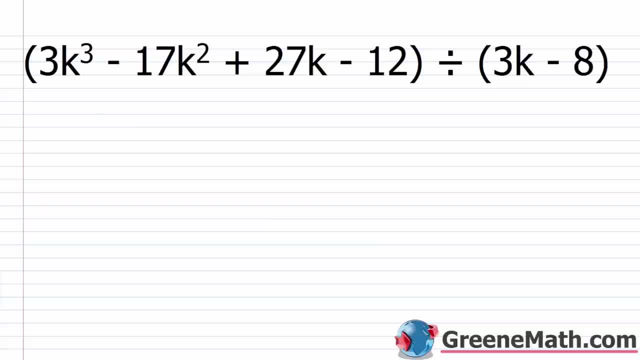 look at that all right so let's take a look at our problem so we have 3k cubed minus 17k squared plus 27k minus 12 and i'm dividing by 3k minus 8 so again this guy goes under the house so 3k cubed minus 17k squared plus 27k minus 12 and we're going to divide this by again 3k minus 8 so i can keep writing this off the top of my head and i'm going to write this off the top of my head and i'm 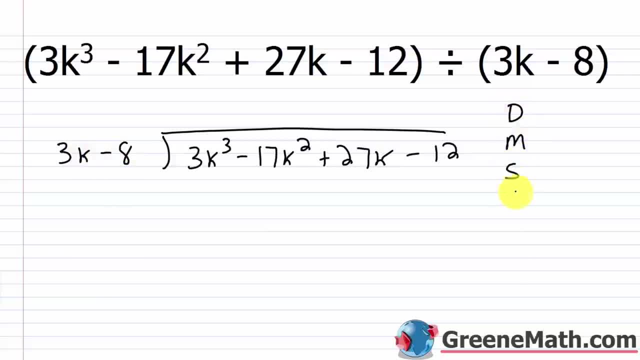 going to put this to the side so division multiplication subtract bring down repeat or remainder so dad mom sister brother rover again first step leading term into leading term so what is 3k cubed over 3k so if i look at this i know the threes are going to cancel and i know k cubed over k is k squared so i'm going to put that over here this is going to be k squared then i'm going to multiply so k squared over k squared is k squared so i'm going to put that over here this is k squared time 3k is 3k cubed k square times negative 8 is minus 8k squared i'm subtracting this line away so this becomes minus this becomes plus 3k cubed minus 3k cubed is zero negative 17k squared plus 8k squared is negative 9k squared then i bring down so bring down the 27k and i'm going to repeat so now i'm going to do again leading term into leading term. So what is negative 9k squared over 3k? Well, this is going to cancel. 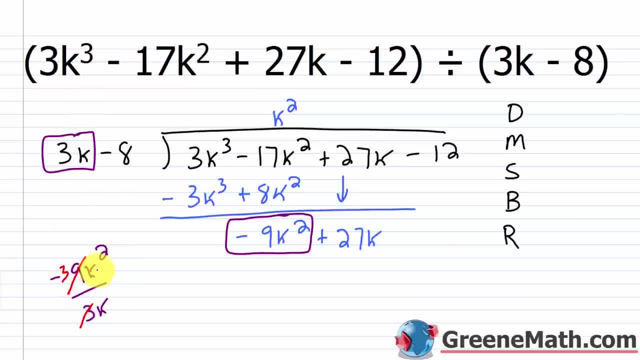 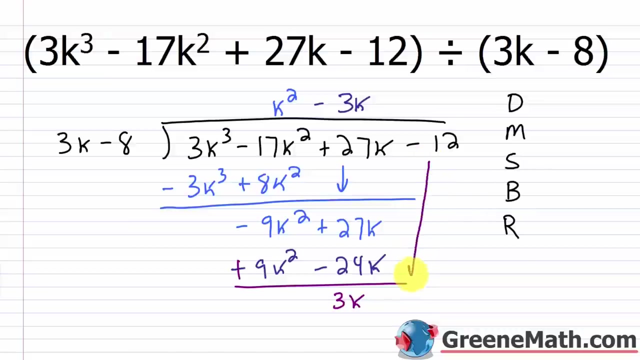 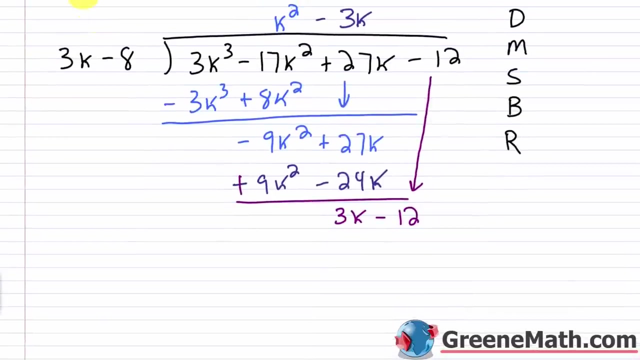 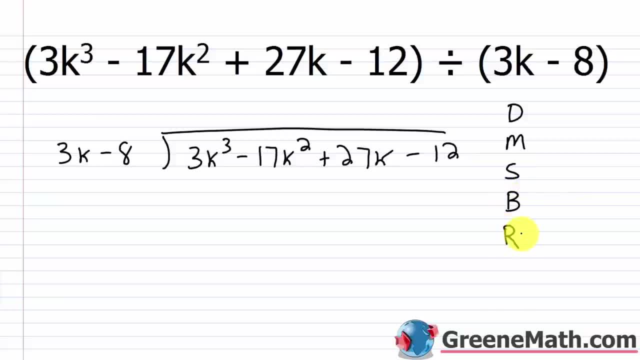 repeat or remainder. So dad, mom, sister, brother, rover, Again, first step, leading term into leading term. So what is 3k cubed over 3k? So if I look at this, I know the 3's. 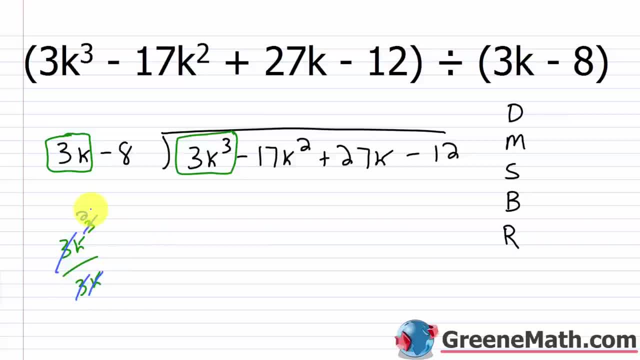 are going to cancel and I know k cubed over k is k squared, So I'm going to put that over here. This is going to be k squared. Then I'm going to multiply, So k squared times 3k is 3k cubed. 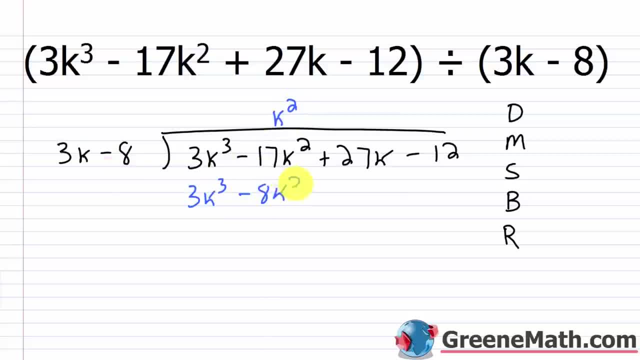 k squared times. negative: 8 is minus 8k squared. I'm subtracting this line away, So this becomes minus. this becomes plus 3k cubed. minus 3k cubed is 0.. Negative: 17k squared plus. 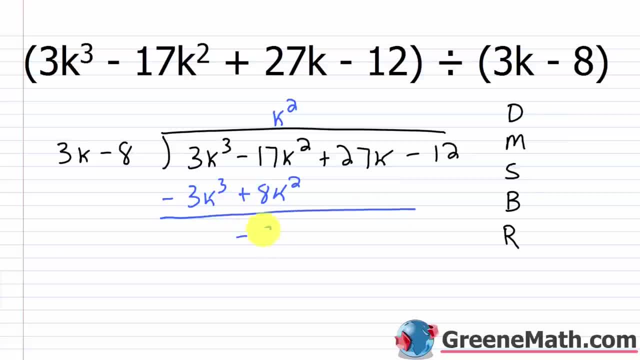 8k squared is negative. 9k squared, Then I bring down. So bring down the 27k And I'm going to repeat. So now I'm going to do again leading term into leading term. So what is negative? 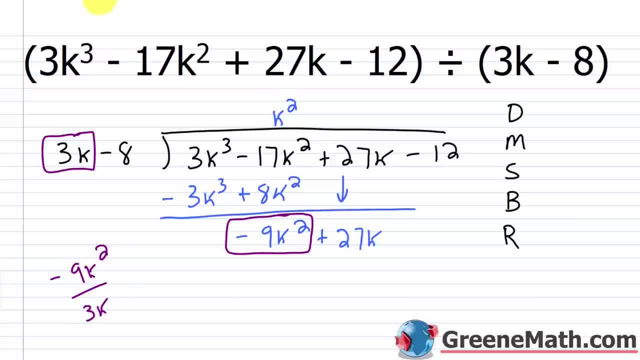 9k squared over 3k. Well, this is going to cancel. Negative 9 over 3 is negative 3.. And then k squared over k is k to the first power. So we get minus 3k. Now again, I'm going to multiply. 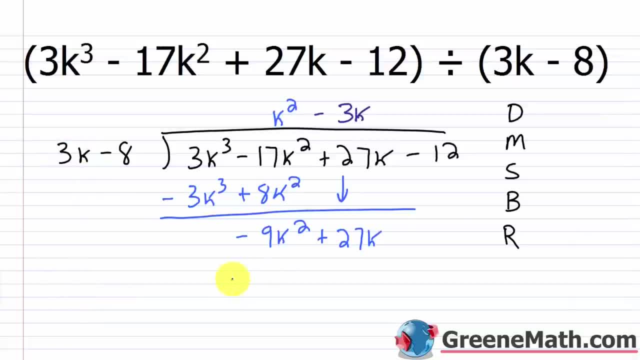 Erase all this. Negative 3k times 3k is negative 9k squared. Negative 3k times negative: 8 is plus 24k. Again, I'm subtracting this away. So what am I going to do? This is going to. 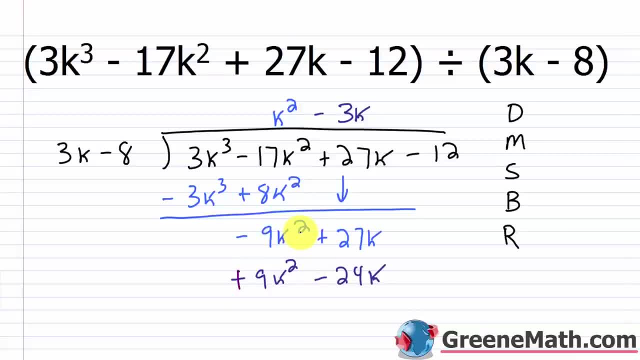 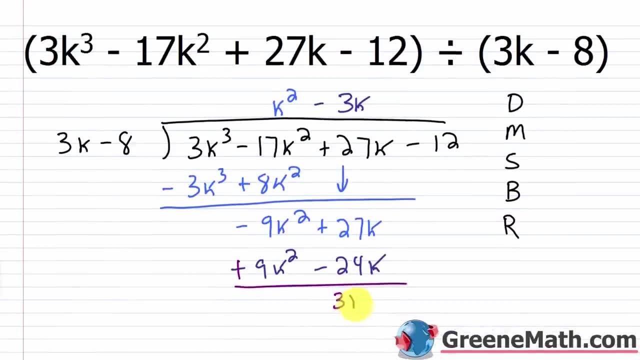 become plus and this is going to become minus. So negative 9k squared plus 9k squared is 0.. 27k minus 24k is 3k. Now I'm going to bring down, So bring down the negative 12.. And 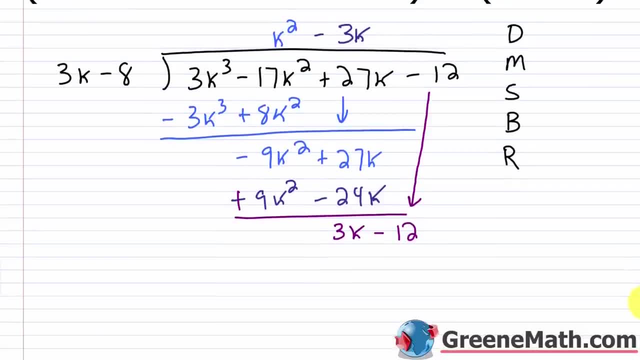 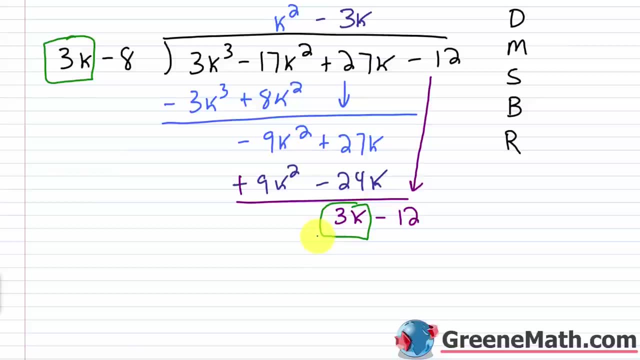 I'm going to repeat, So let me scroll down just a little bit. And so, again, I want to do leading term into leading term. So 3k goes into 3k. We all know that's going to be 1, right, I don't need to write out. 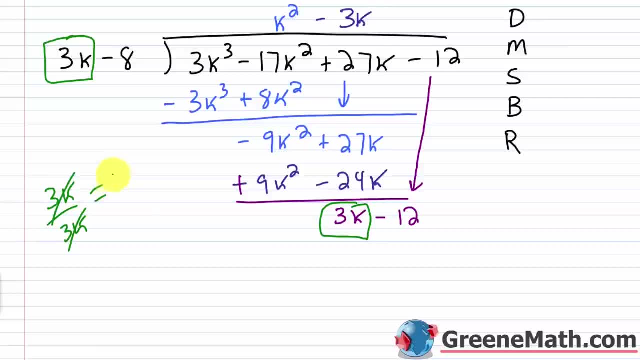 3k over 3k, Same thing over itself as 1.. So plus 1 here, And then I'm going to multiply. So 1 times 3k is 3k. 1 times negative 8 is negative 8.. 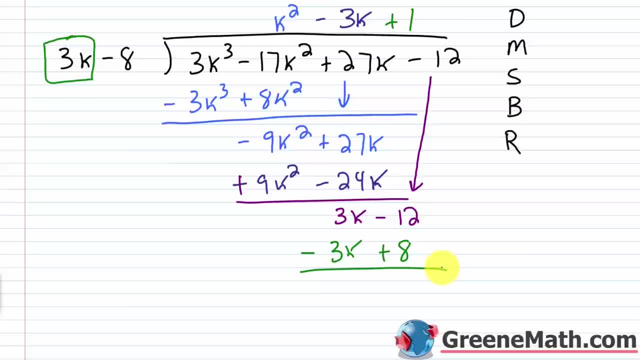 Now I'm subtracting this away, So this becomes minus, This becomes plus. And then look at what's going to happen: 3k minus 3k is 0.. Negative 12 plus 8 is negative 4.. I don't have anything else to bring down here. 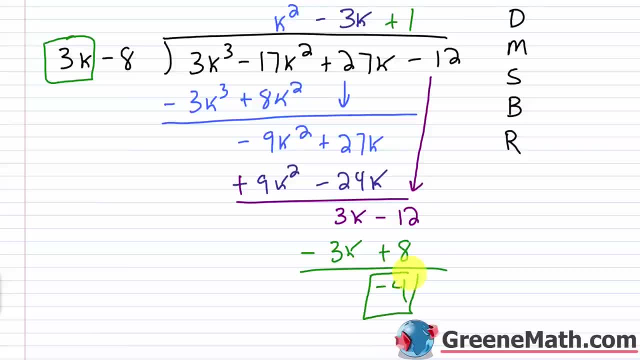 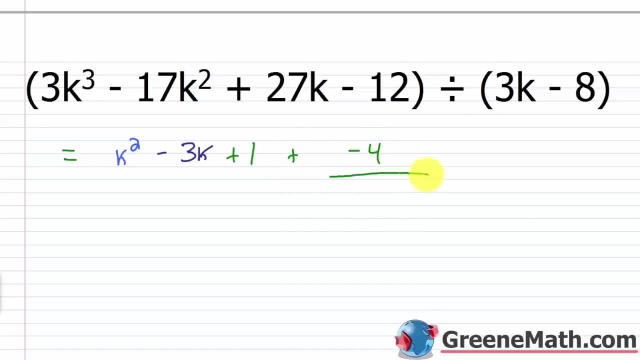 So I'm done. Negative 4 is my remainder. This is the remainder. Okay, So let's erase everything. So I'm going to put equals And then I have that negative 4.. So I'm going to put plus negative 4 over. 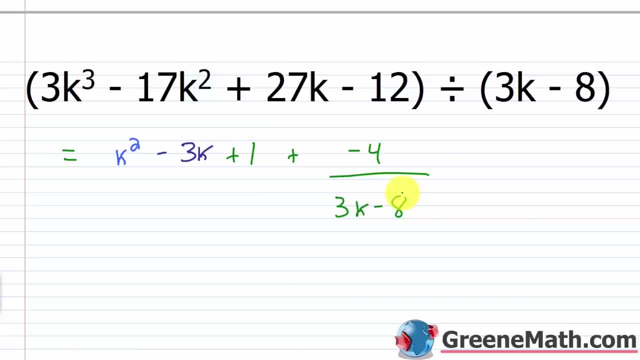 3k minus 8.. Remember, when I divided 50 by 4, I had an answer that was 12 plus. the remainder was 2, right, It was 2 over the divisor of 4.. I just simplified that 2 over 4 is 1 half. 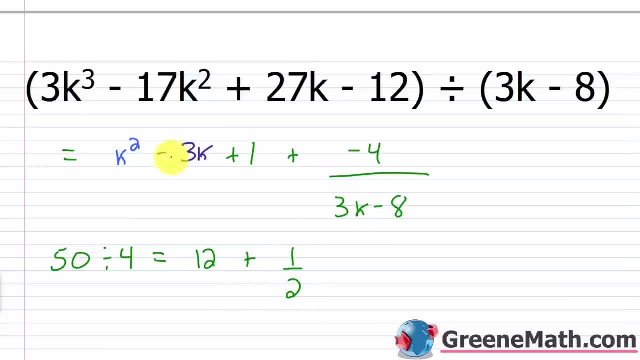 So plus 1 half. This is in the same format as this. All I did was I said plus The remainder over the divisor, So the remainder was negative 4.. The divisor is 3k minus 8. Same as what I did here. The remainder. 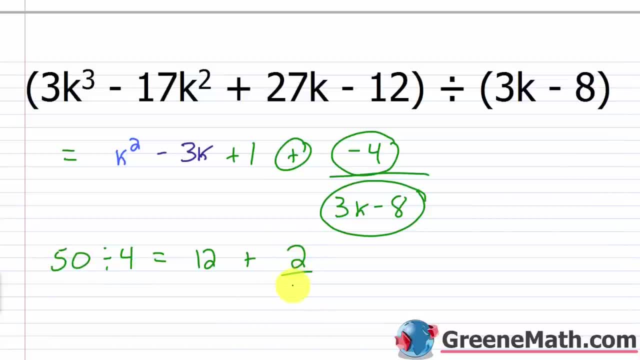 was 2.. And let me kind of write it as 2 fourths so it's not confusing. The remainder was 2.. The divisor is 4.. I just had 1 half, because that's the simplified form, But I'm going. 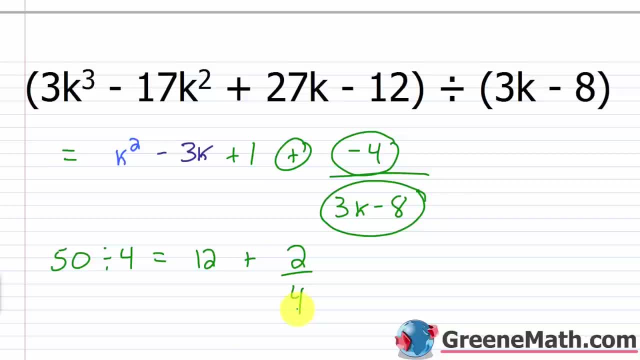 to leave it as 2 fourths right now. So that's how you would go about writing your answer. if you have a remainder, Take the remainder, Put it over the divisor And then you're done. Now to check this Again, it's. 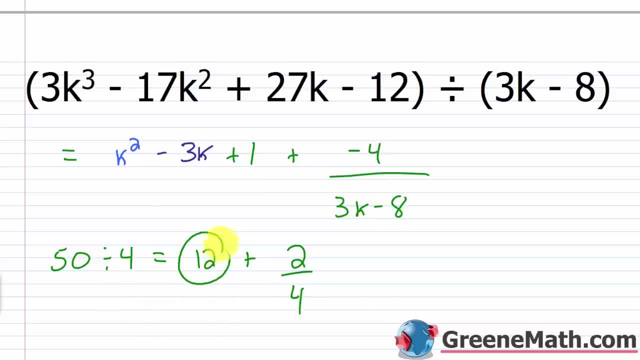 the same thing as when you check this. You can take the quotient, Multiply it by the divisor. So 12 times 4 is 48. And add that remainder of 2. That would get you back to 50.. Or the other. 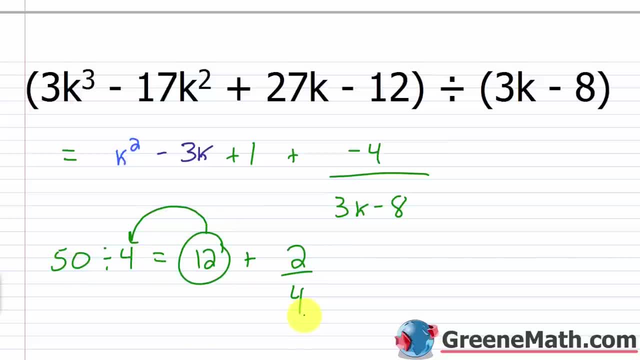 thing I could do is I could multiply 4 by this whole thing, Right? So I'm going to show you both ways here, Just so that we're completely clear on how to check something. So I can kind of just take this part right here and multiply it by this. 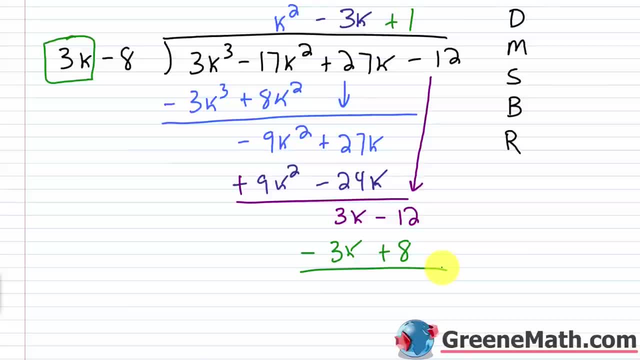 3k minus 3k is 0. Negative 12 plus 8 is negative 4. I don't have anything else to bring down here. So I'm done. 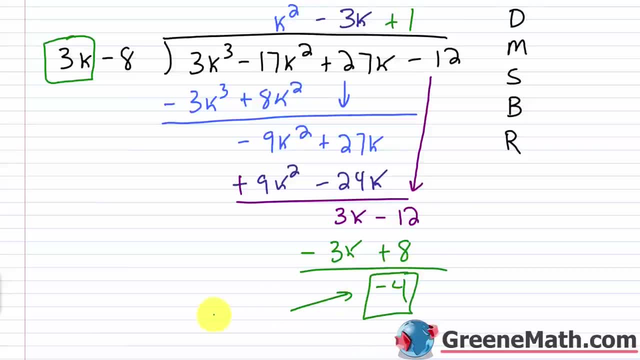 Negative 4 is my remainder. This is the remainder. 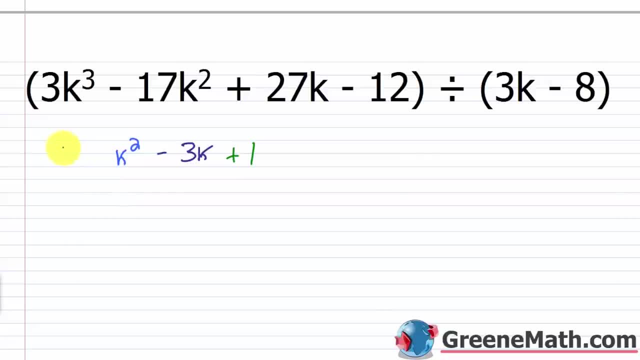 Okay. So let's erase everything. So I'm going to put equals. And then I have that negative 4. So I'm going to put plus negative 4 over 3k minus 8. Remember, when I divided 50, by 4, I had an answer that was 12 plus the remainder was 2, right? It was 2 over the divisor of 4. I just simplified that. 2 over 4 is 1 half. So plus 1 half. This is in the same format as this. All I did was I said plus the remainder over the divisor. So the remainder was negative 4. The divisor is 3k minus 8. Same as what I did here. The remainder was 2. And let me kind of write it as 2 fourths so it's not confusing. The remainder was negative 4 over the divisor of 3k. 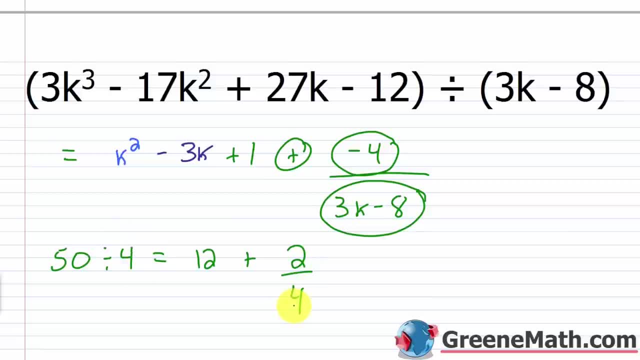 The remainder was negative 4. And let me kind of write it as 2 fourths so it's not confusing. was 2, the divisor is 4. I just had 1 half because that's the simplified form, but I'm going to leave it as 2 fourths right now. So, that's how you would go about writing your answer if you have a remainder. Take the remainder, put it over the divisor, and then you're done. Now, to check this, 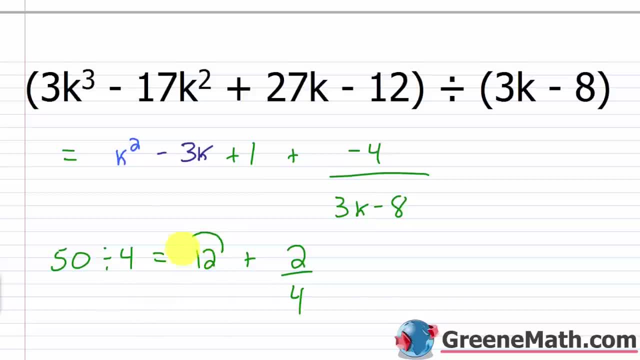 again, it's the same thing as when you check this. You can take the quotient, multiply it by the divisor, so 12 times 4 is 48, and add that remainder of 2. That would get you back to 50. Or, the other thing I could do is I could multiply 4 by this whole thing, right? So, I'm going to show you both ways here, just so that we're completely clear on how to check something. So, I can kind of just take this part right here and multiply it by this part right here, and when I'm done, just add negative 4, and that'll give me this. So, in other words, if I took 3k minus 8, and I multiplied it by k squared minus 3k plus 1, 3k is 2. 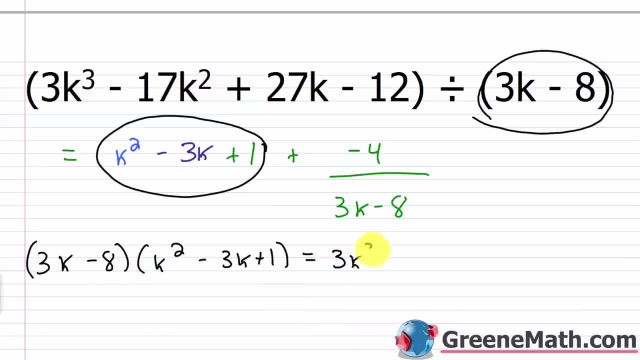 3k is 1. k times k squared is 3k cubed. 3k times negative 3k is minus 9k squared. 3k times 1 is plus 3k. Then negative 8 times k squared is minus 8k squared. Negative 8 times negative 3k is plus 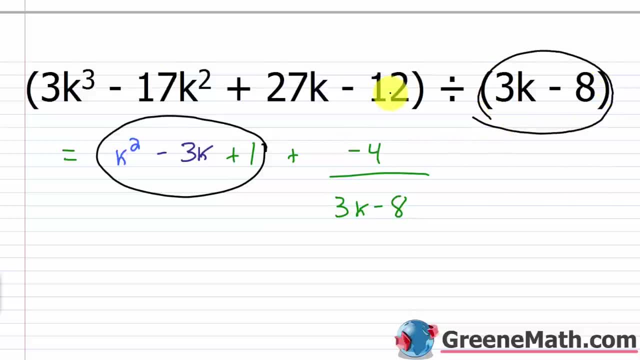 part right here And when I'm done, just add negative 4 and that will give me this. In other words, if I took 3k minus 8 and I multiplied it by k squared minus 3k plus 1, 3k times k squared is: 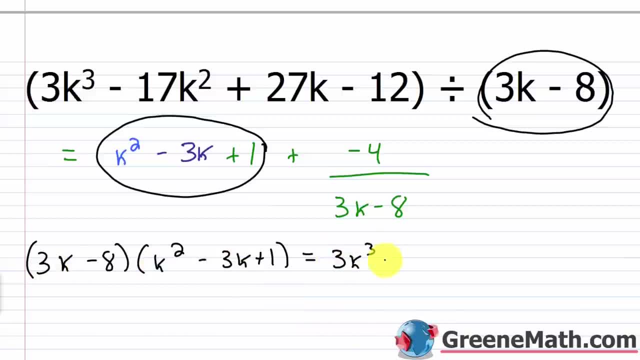 3k cubed: 3k times negative 3k is minus 9k squared 3k times 1 is plus 3k. Then negative 8 times k: squared is minus 8k squared. Negative, 8 times negative 3k is: 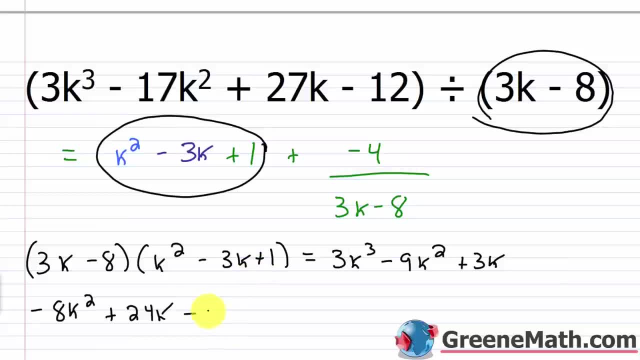 plus 24k. Negative 8 times 1 is negative 8.. So combining like terms here, negative 9k squared minus 8k squared would be negative 17k squared. Then 3k plus 24k is 27k. 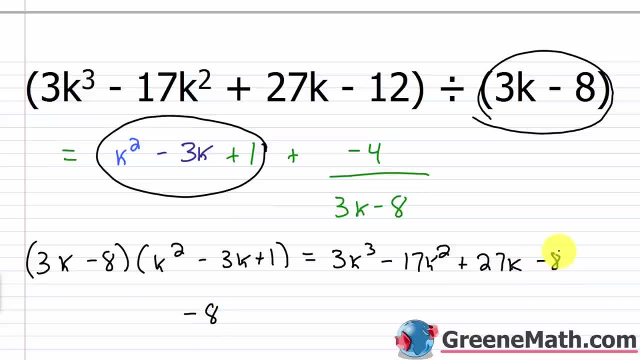 And then I have that minus 8 there. So if I look at my answer here, 3k cubed minus 17k squared plus 27k minus 8, it's the same thing as this. the only difference is this minus 8 here. 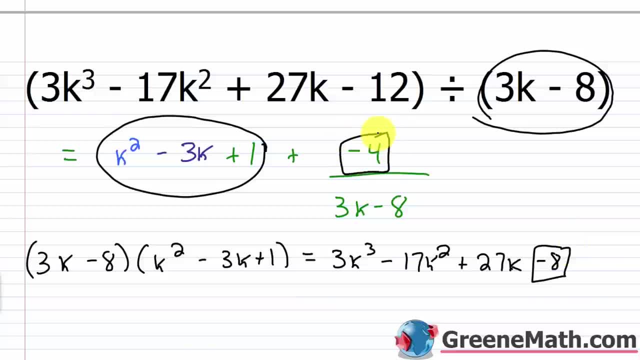 So why do you think that is? Again, the remainder was negative 4.. So if I added a negative 4, if I said, hey, this minus another 4, this would end up being negative 12, just like it is right there. 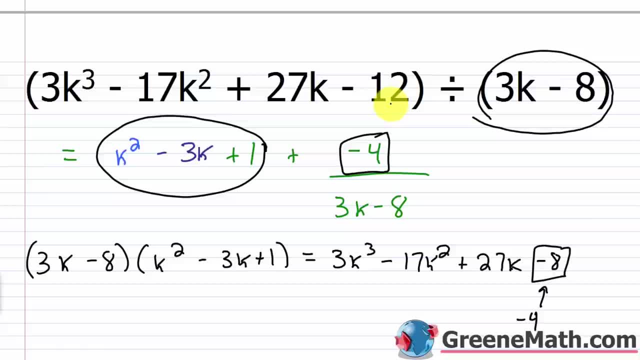 And you get your original dividend back. Now let me show you the other way. So you could also multiply 3k minus 8 times this whole thing, k squared minus 3k plus 1 plus negative 4 over 3k minus. 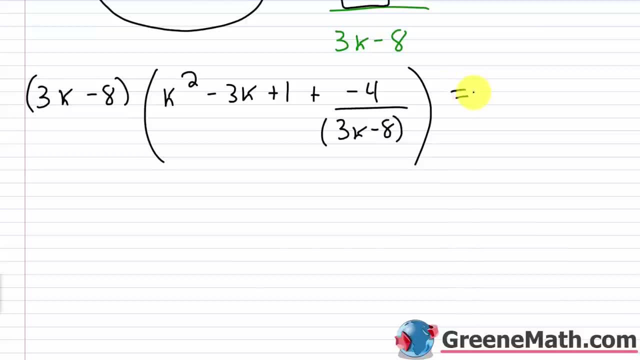 8.. Let me just kind of do this a different way. Let me go. we'll have k squared times 3k minus 8.. I'm just distributing this to each term And then I'll have negative 3k, or I could. 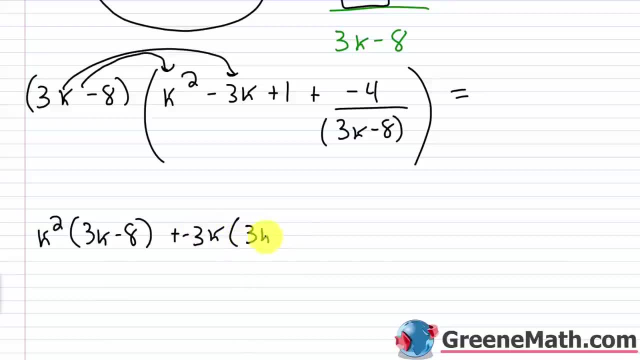 put plus negative 3k, like that times 3k minus 8. And then we'll distribute this again, So we'd have 1 times 3k minus 8.. That's just 3k minus 8. And then let's distribute it one more time. 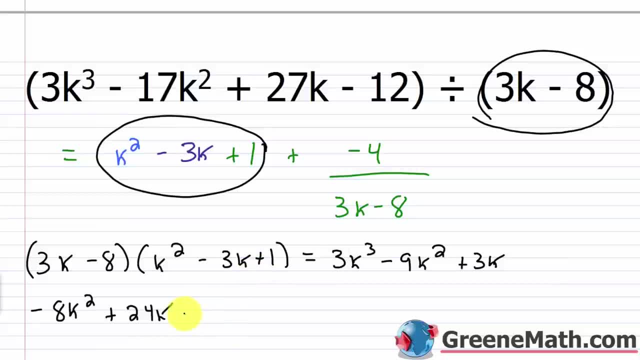 24k. And then negative 8 times 1 is negative 8. So combining like terms here, negative 9k squared minus 8k squared would be negative 17k squared. Then 3k plus 24k is 27k. 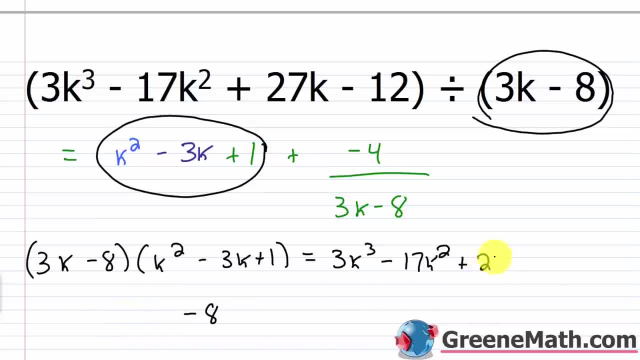 And then I have that minus 8 there. So if I look at my answer here, 3k cubed minus 17k squared 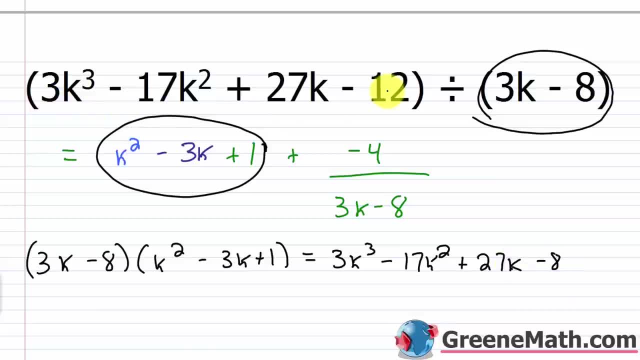 plus 27k minus 8, it's the same thing as this. The only difference is this minus 8 here. So why do you think that is? Again, the remainder was negative. So I'm going to take that minus 8 and negative 4. So if I added a negative 4, if I said, hey, this minus another 4, this would end up being negative 12, just like it is right there. And you get your original dividend back. Now, 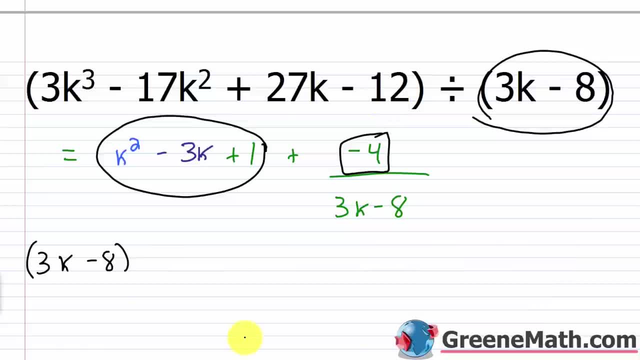 let me show you the other way. So you could also multiply 3k minus 8 times this whole thing. 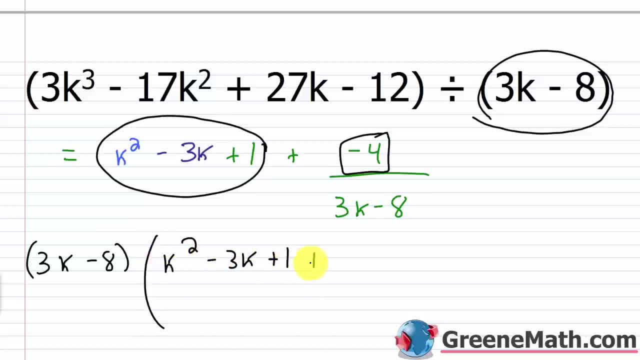 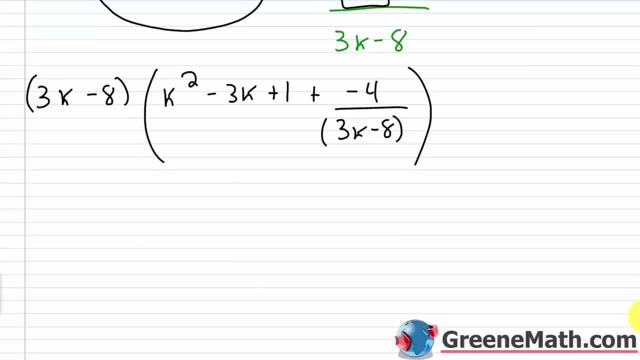 k squared minus 3k plus 1 plus negative 4 over 3k minus 8. Let me just kind of do this. 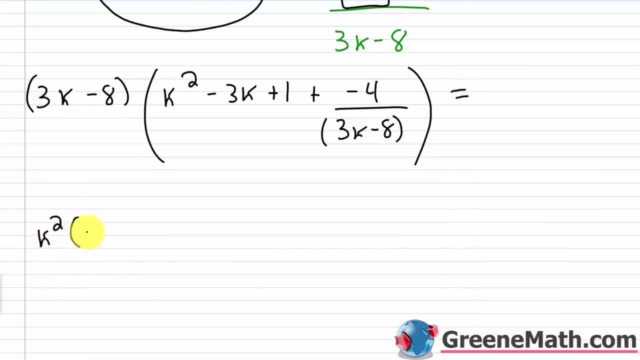 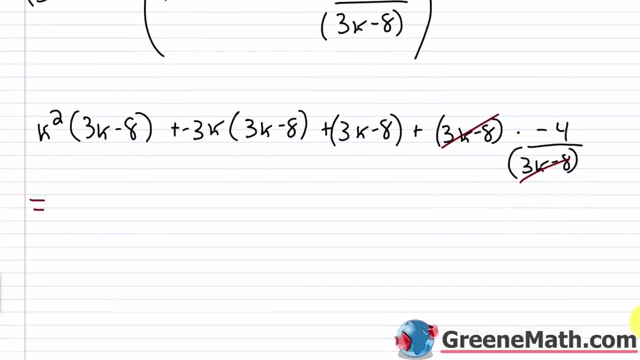 Let me go. We'll have k squared times 3k minus 8. I'm just distributing this to each term. And then I'll have negative 3k, or I could put plus negative 3k like that, times 3k minus 8. And then we'll distribute this again. So we'd have 1 times 3k minus 8. That's just 3k minus 8. And then let's distribute it one more time. What you'd have here is plus 3k minus 8 times negative 4 over 3k minus 8. So these two are going to cancel themselves out. It's the same thing over itself. And so I'm just left with a negative 4. So if I put equals here, let me kind of go through this. k squared times 3k is 3k cubed. k squared times negative 8 is minus 8k squared. 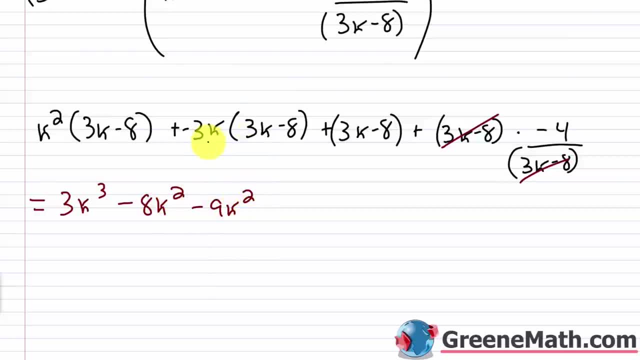 Then negative 3k times 3k is minus 9k squared. Negative 3k times negative 8 is plus 24k. Then I have 3k minus 8, so plus 3k minus 8. And then after we canceled this, we ended up with just plus negative 4. So what you're going to find here is that you get your dividend back exactly. 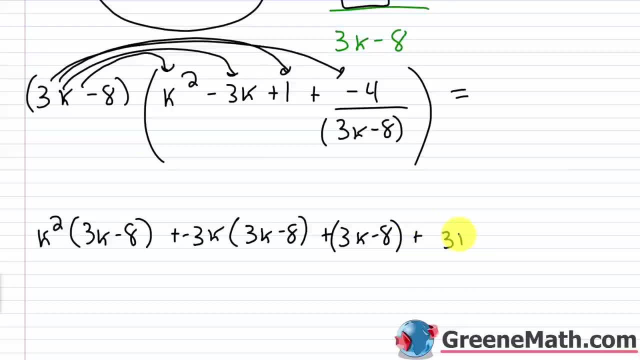 What you'd have here is plus 3k minus 8, times negative 4 over 3k minus 8.. So these two are going to cancel themselves out. It's the same thing over itself, And so I'm just left with a negative. 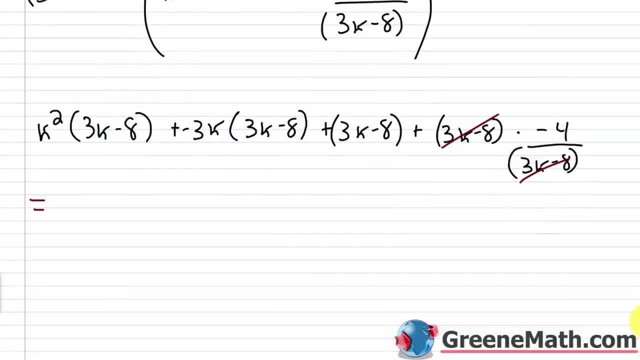 4. So if I put equals here, let me kind of go through this: k squared times 3k is 3k cubed k squared times negative, 8 is minus 8k squared. Then negative 3k times 3k is minus 9k squared. 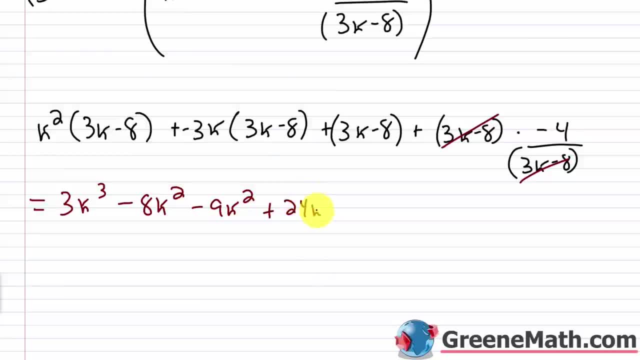 Negative 3k times negative. 8 is plus 24k. Then I have 3k minus 8,, so plus 3k minus 8.. And then, after we cancelled this, we ended up with just plus negative 4.. So what you're going to find here is that you get your. 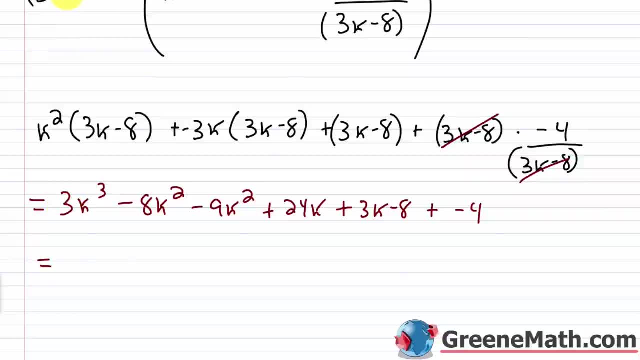 dividend back. exactly So 3k cubed, 3k cubed negative, 8k squared minus 9k squared is minus 17k squared, Then 24k plus 3k, that's plus 27k, And then 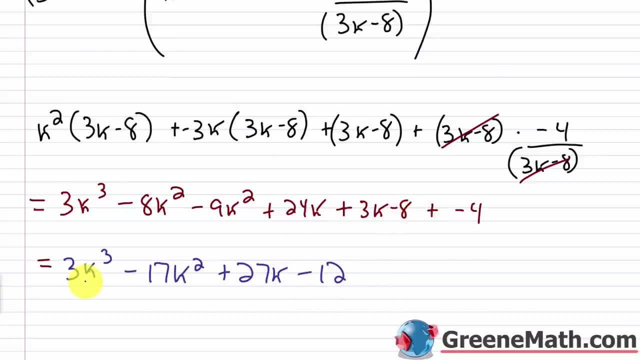 negative 8 plus negative 4 is negative 12.. So I get 3k cubed minus 17k squared plus 27k minus 12,, which is exactly the dividend that I started with. Hello and welcome to Algebra 1, Lesson 35.. 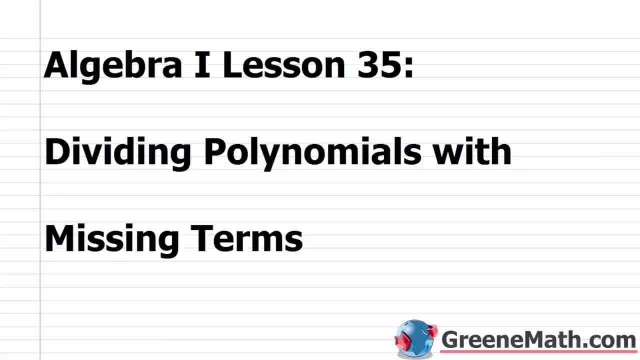 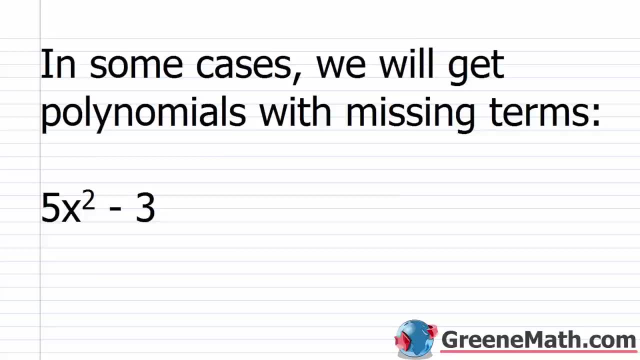 In this video we're going to learn about dividing polynomials with missing terms. So somewhere in your section on dividing polynomials you're going to get this kind of subsection that talks about dividing polynomials with missing terms. It's not any more difficult. 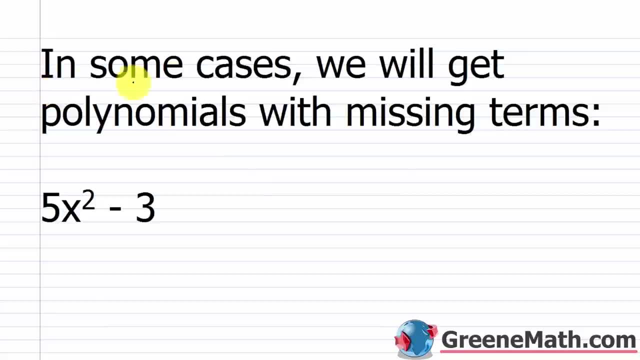 Basically, what you're looking at is that in some cases we will get polynomials with missing terms, And what I mean by that. if you look at this kind of first example here we see 5x squared minus 3.. So if my highest power 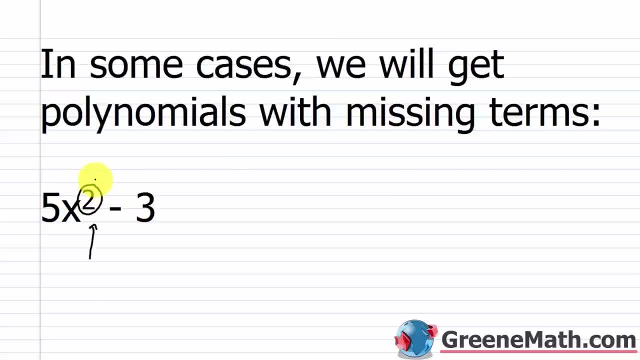 on x is a 2, then I've got to go down kind of in order. So in other words, I need an x to the first power there, and I don't have it. That's what I mean by a missing term. 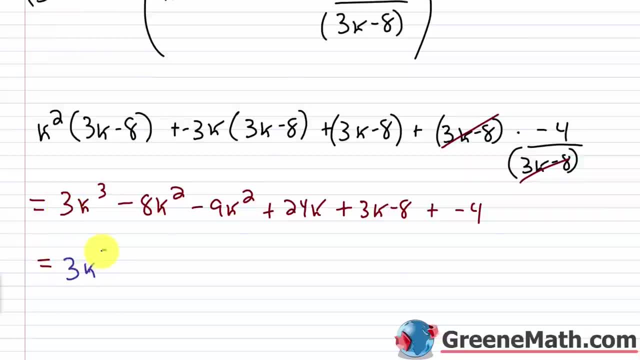 So 3k cubed, 3k cubed, negative 8k squared minus 9k squared is minus 17k squared. Then 24k plus 3k, that's plus 27k. And then negative 8 plus negative 4 is negative 12. So I get 3k cubed minus 17k squared plus 27k squared. Minus 12, which is exactly the dividend that I started with. 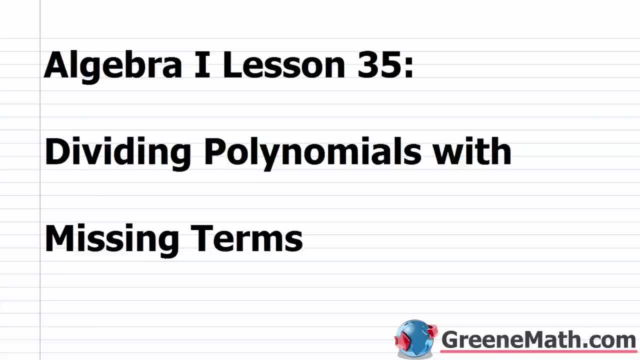 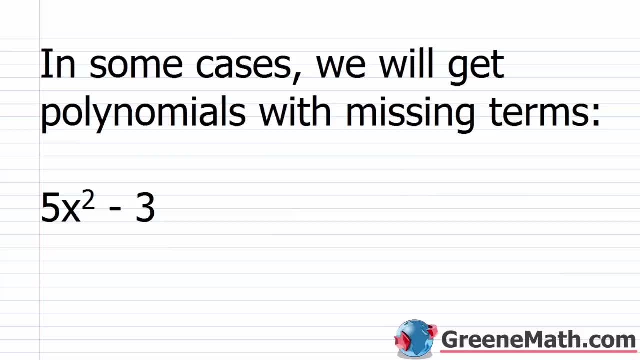 Hello and welcome to Algebra 1 Lesson 35. In this video, we're going to learn about dividing polynomials with missing terms. So somewhere in your section on dividing polynomials, you're going to get this kind of subsection that talks about dividing polynomials with missing terms. It's not any more difficult. Basically, what you're looking at is that in some cases, we will get polynomials with missing terms. So in this case, we're going to get polynomials with missing terms. And what I mean by that, if you look at this kind of first example here, we see 5x squared minus 3. So if my highest power on x is a 2, then I've got to go down kind of in order. So in other words, I need an x to the first power there, and I don't have it. That's what I mean 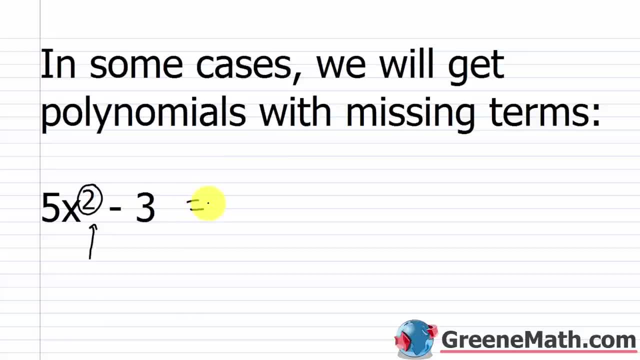 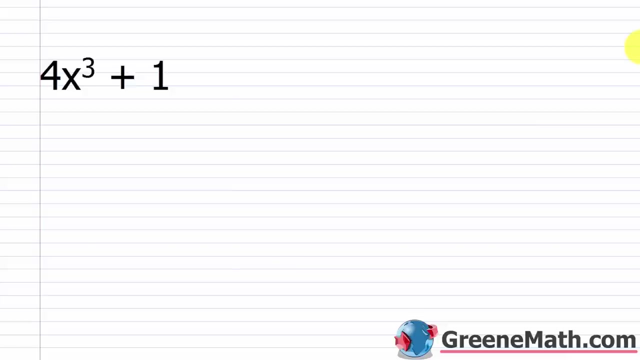 by a missing term. So we have a little trick for that. We rewrite this as 5x squared plus 0 as the missing term. The missing term was x to the first power, x to the first power, and then we have minus 3. Remember, 0 times anything is 0. So legally, I can do that, and these two things are the same. I haven't changed the value. We just made it look a little bit different. Remember that 0 is used in our number system as a placeholder. And it's so different here. It's just being used as a placeholder. For example, in a number like this, I'm going to use a placeholder. And I'm going to write like 1,007. I have 1,007. These zeros here are just placeholders. They're telling me that I have 0 hundreds and I have 0 tens. It is the same thing. I have 0x to the first power here. So the 0 is just nothing more than a placeholder. But look at something like 4x cubed plus 1. Again, 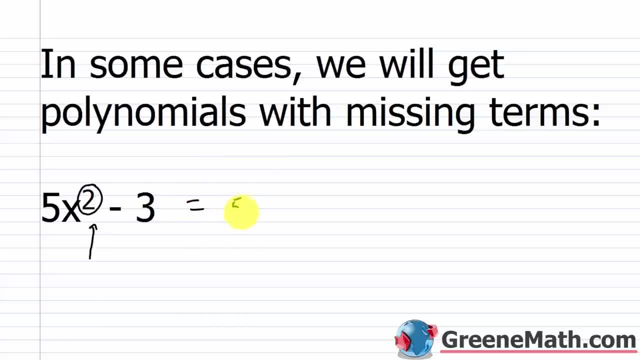 We have a little trick for that. We rewrite this as 5x squared plus 0 as the coefficient for the missing term. The missing term was x to the first power, x to the first power, And then we have minus 3.. 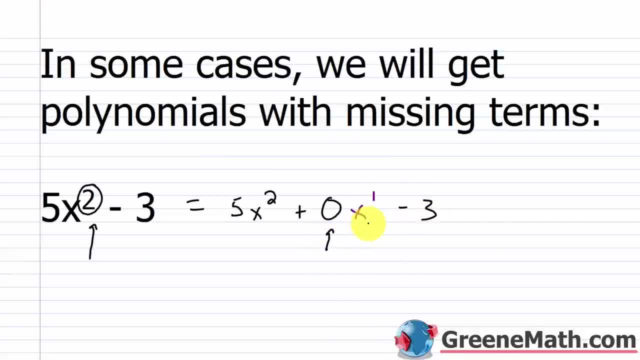 Remember, 0 times anything is 0. So legally I can do that and these two things are the same. I haven't changed the value. We just made it look a little bit different. Remember that 0 is used in our number system as a. 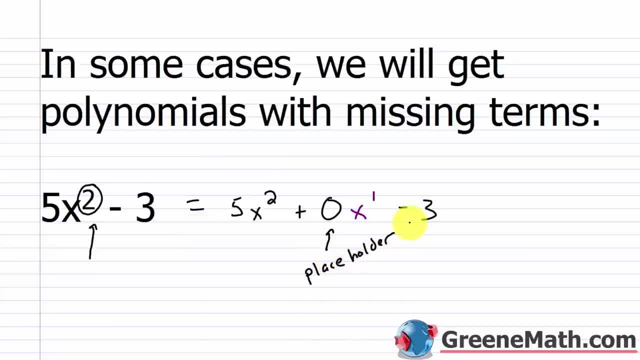 placeholder And it's so different. here It's just being used as a placeholder, For example, in a number like 1,007.. I have 1,007.. These zeros here are just placeholders. They're telling me that I have. 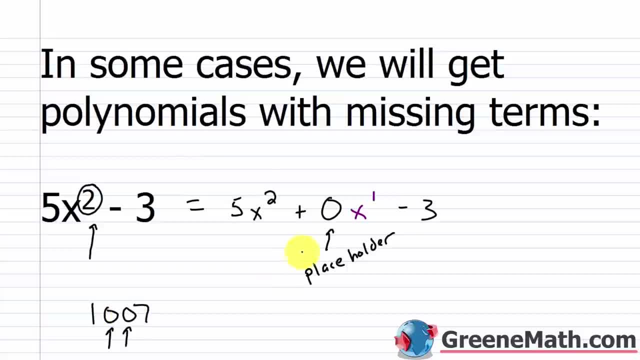 0 hundreds and I have 0 tens. It is the same thing. I have 0 x to the first power here, So the 0 is just nothing more than a placeholder. But look at something like 4x cubed plus 1.. 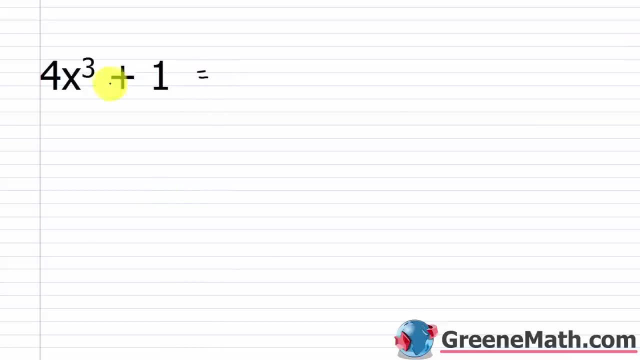 Again, if I'm looking for what's missing. I want you to think about this carefully: The highest power on x is a 3. We have x cubed, So I'm missing x squared and I'm missing x to the first power, So I can rewrite. 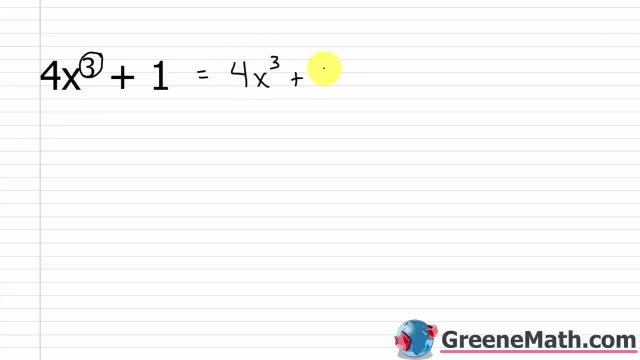 this as 4x cubed plus 0 x squared, plus 0 x to the first power And then finally plus 1.. So I have 0 as a placeholder and 0 as a placeholder. I have 0 x squared and 0 x. 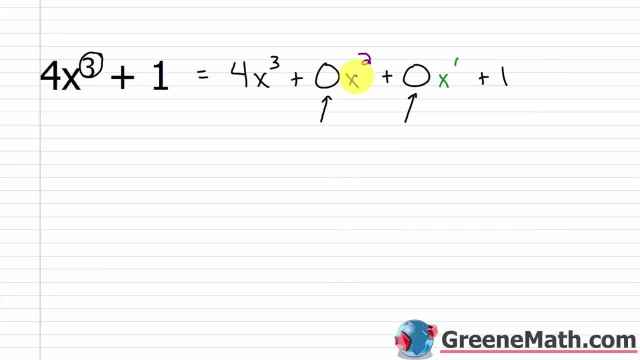 to the first power. So I'm representing them, but with 0 as the coefficient, because, again, 0 times anything is 0.. So the basic idea here is, when performing long division with polynomials with missing terms, we need to use 0. 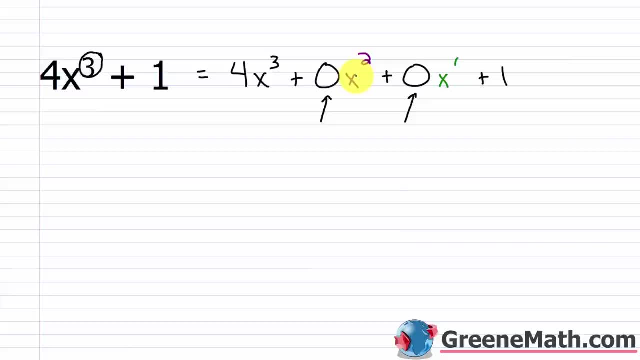 as the coefficient for each missing term, And if something's written in standard form, it's very, very easy to see what's missing. If I have 4x cubed plus 1, I know I'm missing an x squared and an x to the first power. If I 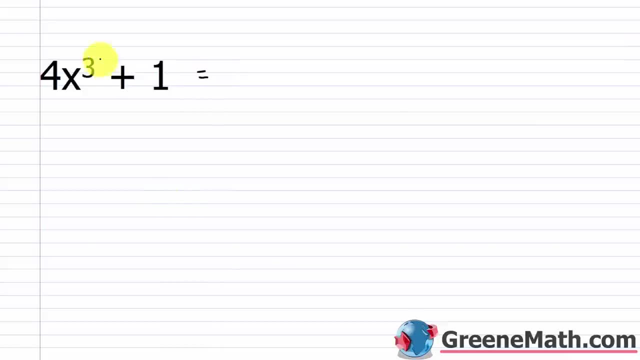 if I'm looking for what's missing, I want you to think about this carefully. The highest power on So I'm missing x squared and I'm missing x to the first power. So I can rewrite this as 4x cubed plus 0x squared plus, next I'd do 0x to the first power, and then finally plus 1. 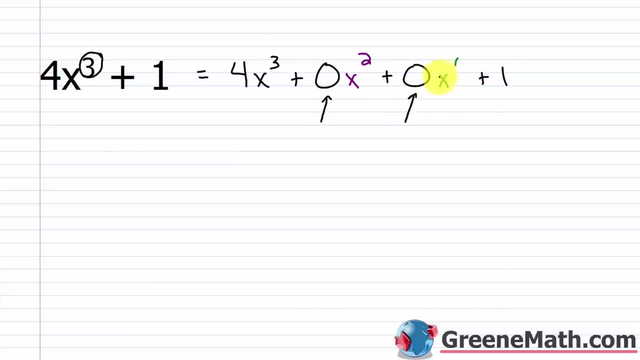 So I have 0 as a placeholder and 0 as a placeholder. I have 0x squared and 0x to the first power. So I'm representing them, but with 0 as the coefficient, because again, 0 times anything is 0. 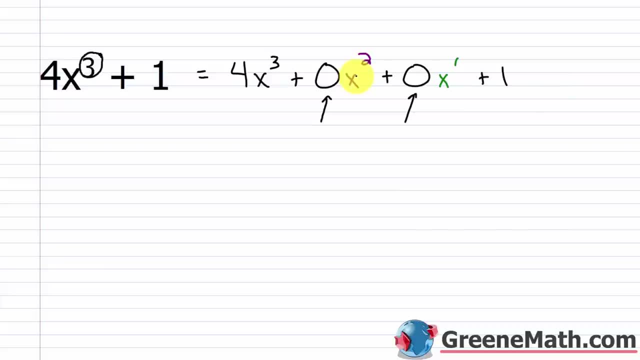 So the basic idea here is when performing long division with polynomials with missing terms, we need to use 0 as the coefficient for each missing term. And if something's written in standard form, it's very, very easy to see what's missing. 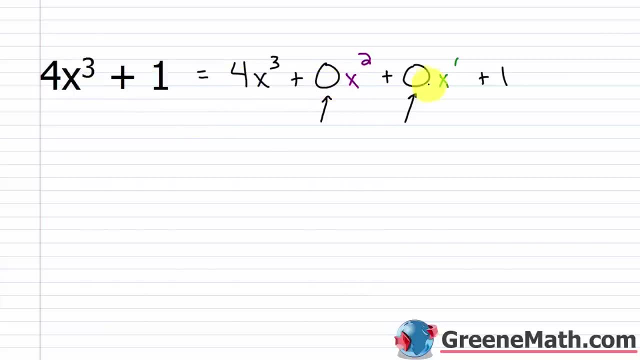 If I have 4x cubed plus 1, I know I'm missing an x squared and an x to the first power. If I had something like, let's say 7. If I had something like 7x to the sixth power minus 2, well, my highest power on x is the sixth power. So I'm missing x to the fifth power, fourth power, third power, squared, and first power. And a lot of times you're not going to have that many missing powers. 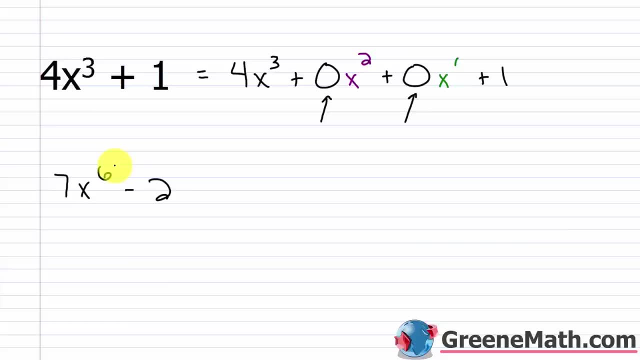 You'll just have, you know, one or two here or there. Like I had two here. 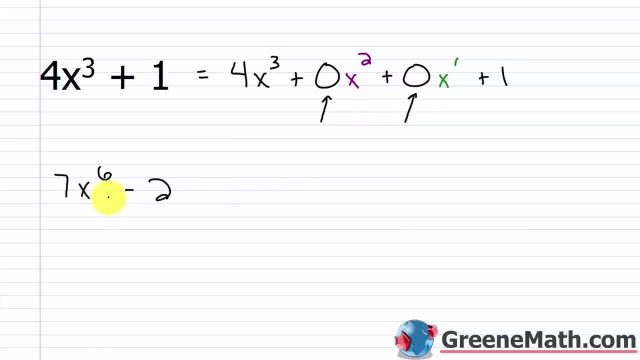 You know, in this instance, you'd have the fifth power, the fourth power, the third power, the second power, and the first power. There'd be five missing powers. It'd be a lot for your teacher to throw at you. You'll probably just get one or two. So let's take a look at an example. 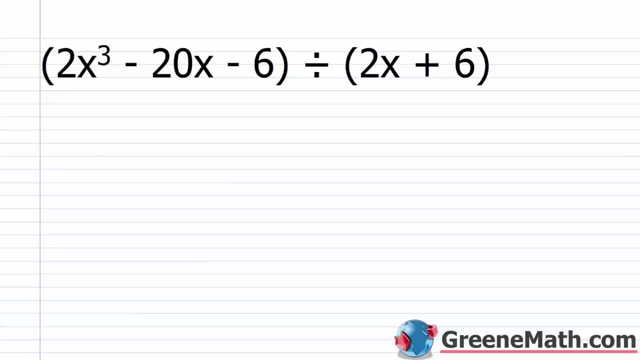 Again, this is not any more difficult than dividing with polynomials when you have all the terms. It's the same kind of setup. 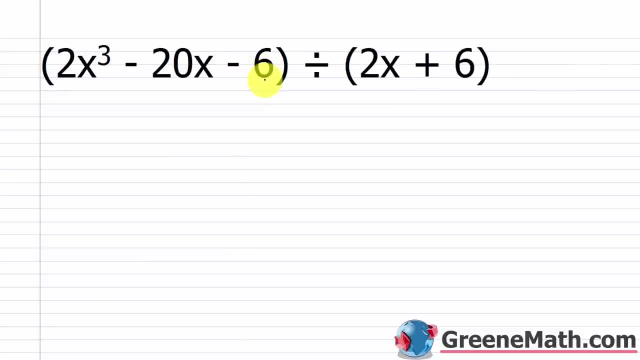 So I have 2x cubed minus 20x minus 6. That is my dividend. So remember that goes, as we say, underneath the house. So 2x cubed. I have minus 20x next. So I'm missing that x squared term. So I'm going to put plus 0x squared as a placeholder. And then minus 20x. And then minus 6x. 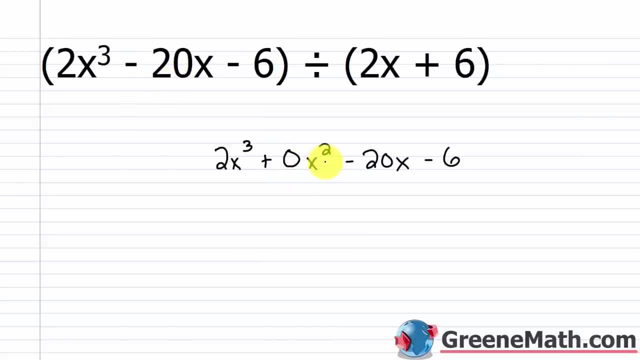 Again, if you're missing that x squared term, you just put 0x squared. That's all you need to do. All right. 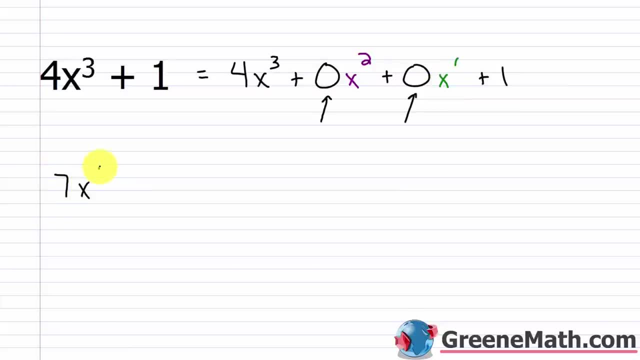 had something like, let's say, 7x to the sixth power minus 2,. well, my highest power on x is the sixth power, So I'm missing x to the fifth power, fourth power, third power squared and first power, And a lot of times you're not. 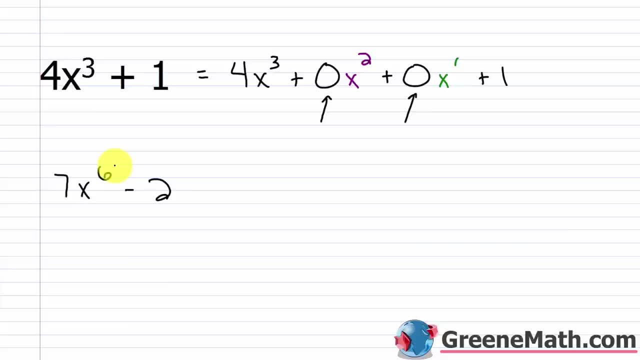 going to have that many missing powers. You'll just have one or two here or there, Like I had two here. In this instance, you'd have the fifth power, the fourth power, the third power, the second power and the first power. 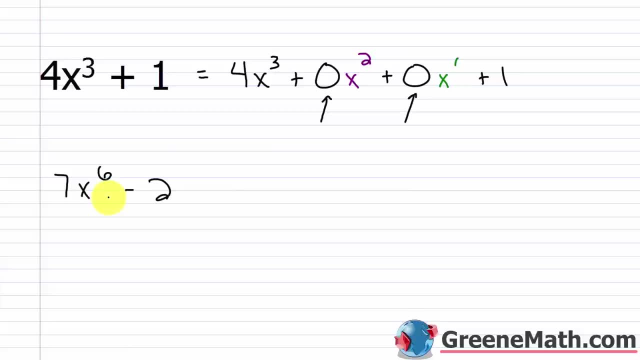 There'd be five missing powers. It'd be a lot for your teacher to throw at you. You'll probably just get one or two. So let's take a look at an example. Again, this is not any more difficult than dividing with polynomials when you have 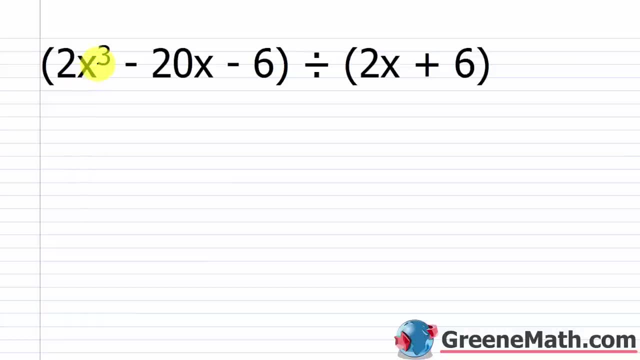 all the terms. It's the same kind of setup. So I have 2x cubed minus 20x minus 6.. That is my dividend. So remember that goes, as we say, underneath the house. So 2x cubed. 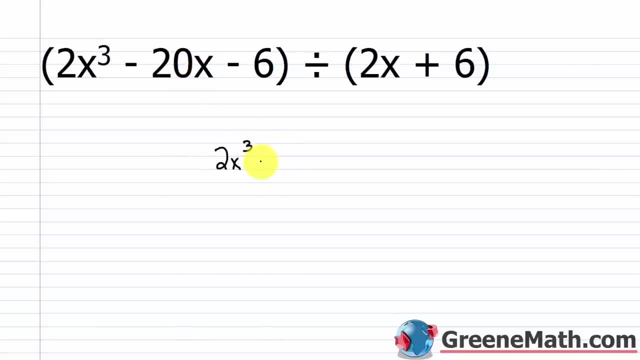 I have minus 20x next. So I'm missing that x squared term. So I'm going to put plus 0x squared as a placeholder, And then minus 20x and then minus 6.. Again, if you're missing that x squared term, 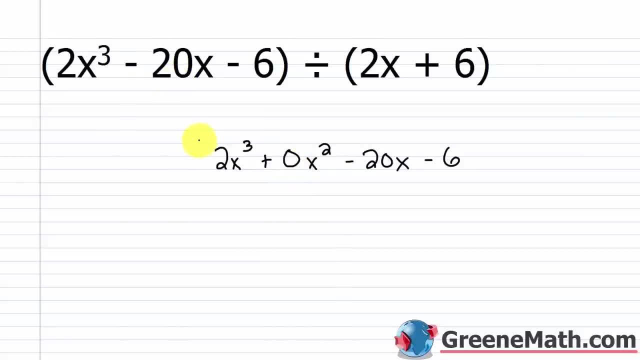 you just put 0x squared. That's all you need to do, Alright, so then we're going to set this up Out here: my divisor 2x plus 6.. And once you've done that, again it's the same thing. 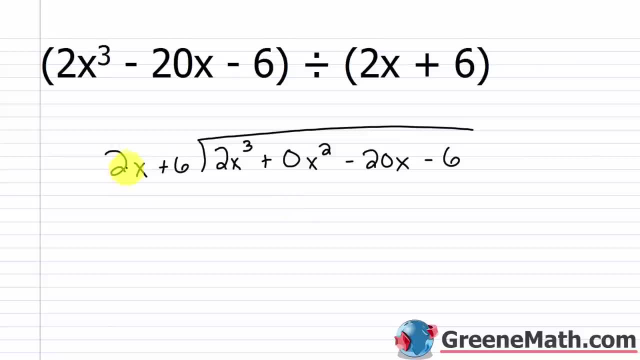 that you've been doing throughout this section. You're going to go leading term into leading term. So 2x goes into 2x cubed. how many times? So what is 2x cubed over 2x? We know that these 2s are going to cancel completely. 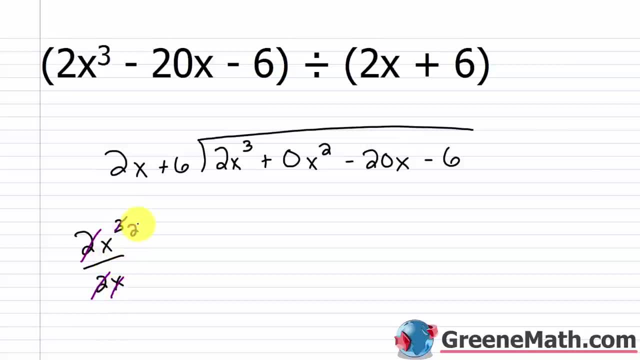 x cubed over x. we know this is going to be x squared, So I'm going to put x squared over this guy right here. This is where I'm going, And then I'm going to multiply. So let me erase this real quick. 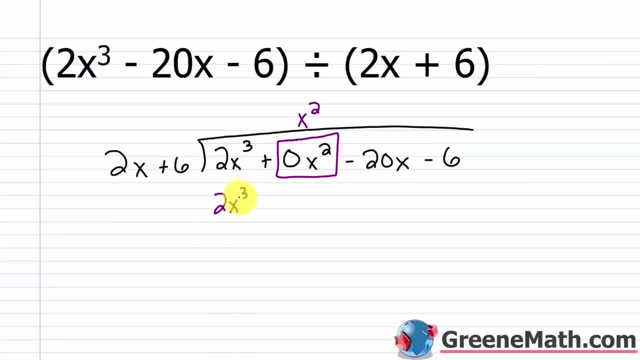 x squared times 2x is 2x cubed. Then x squared times 6 is plus 6x squared. Now again, I want to subtract away this polynomial, And I know, in the last kind of section where we just talked about dividing. 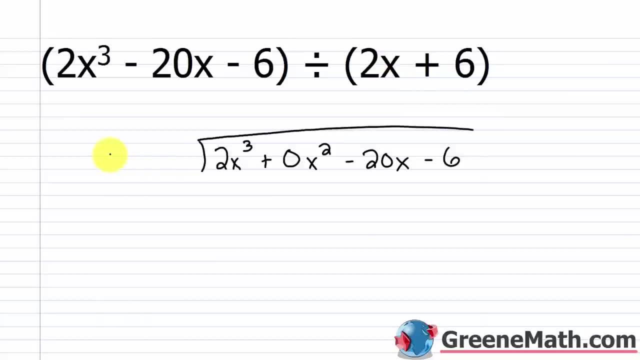 So then we're going to set this up. Out here, my divisor, 2x plus 6. And once you've done that, again, it's the same thing that you've been doing throughout this section. 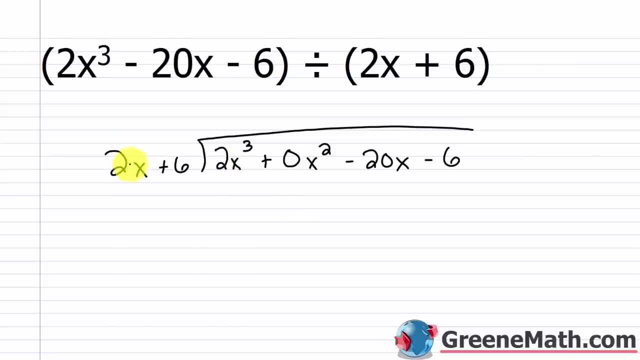 You're going to go leading term into leading term. So 2x goes into 2x cubed how many times? So what is 2x cubed over 2x? We know that these 2s are going to cancel completely. x cubed over x, we know this is going to be x squared. 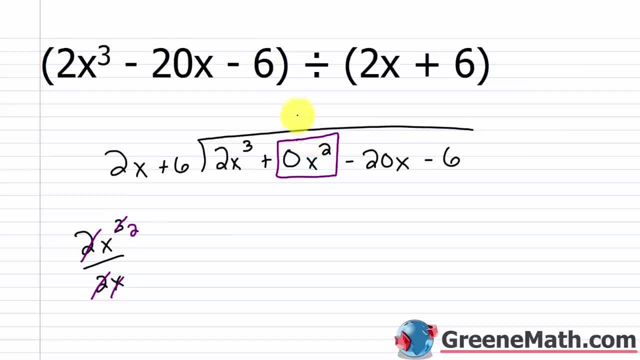 So I'm going to put x squared over this guy right here. This is where I'm going. And then I'm going to multiply. 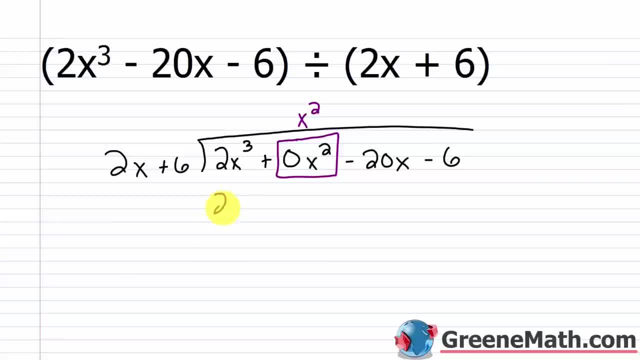 So let me erase this real quick. x squared times 2x is 2x cubed. 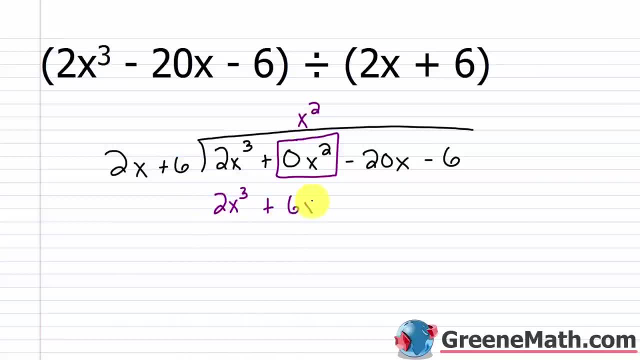 Then x squared times 6 is plus 6x squared. 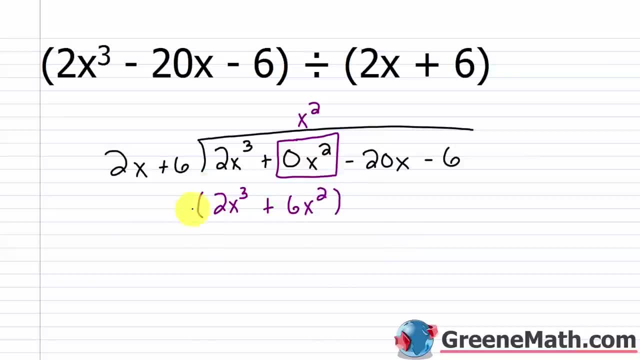 Now, again, I want to subtract away this polynomial. And I know in the last kind of section where we just talked about dividing polynomials, 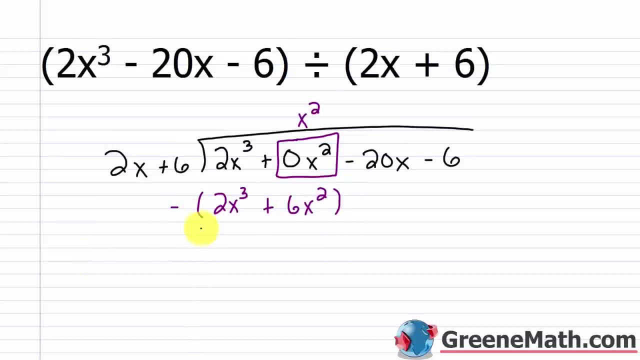 I kind of got you to the point to where, I didn't go through and do this extra step of putting parentheses around it, putting a minus in front, and then erasing all this and changing the signs. 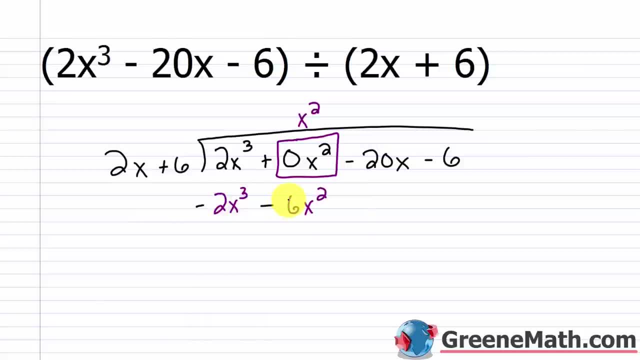 Again, once you get comfortable, just change your signs and move on. 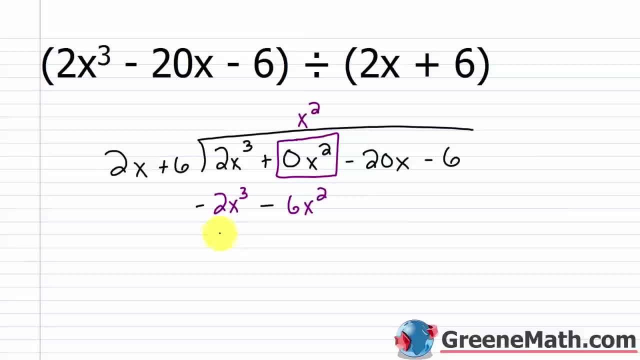 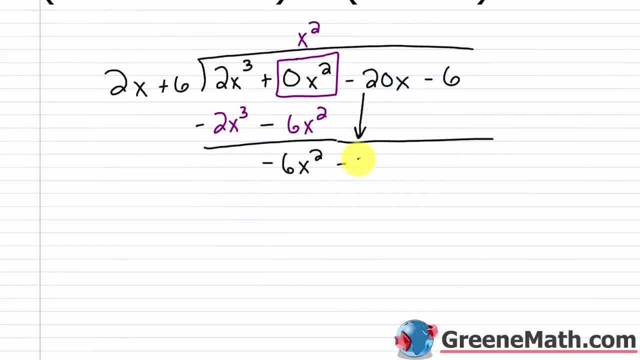 Right now, I'm just going to add. 2x cubed plus negative 2x cubed is 0. 0x squared minus 6x squared is minus or negative 6x squared. Scroll down, get a little room going. All right, now I'm going to bring down my next term. And my next term is a negative 28. And then again, I'm going to go leading term into leading term. So what is negative 6x squared over 2x? We know that this is going to cancel with this and give me a negative 3. And x squared will cancel with x. That'll give me x to the first power. So I'm going to have a minus 3x. 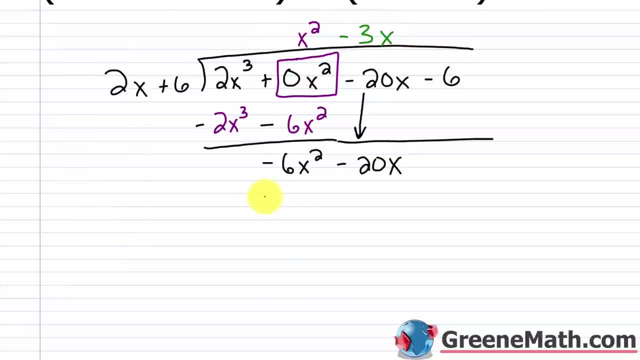 And I'm going to multiply. Negative 3x times 2x is negative 6x squared. 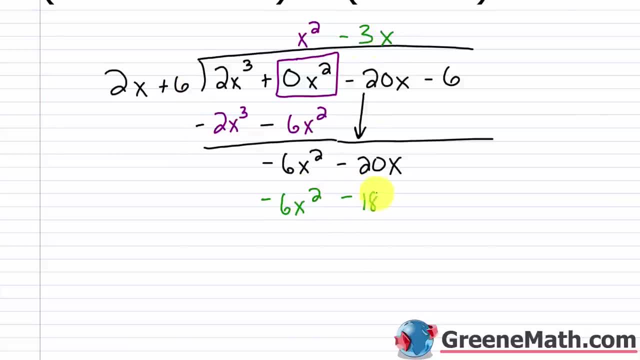 Negative 3x times 6 is negative 18x. 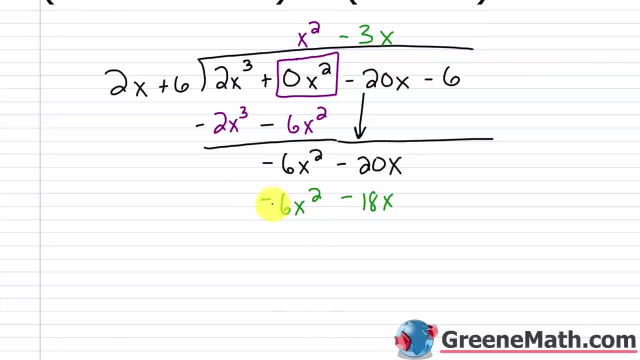 And again, I want to change the sign of each term here because I'm going to subtract this bottom one away. 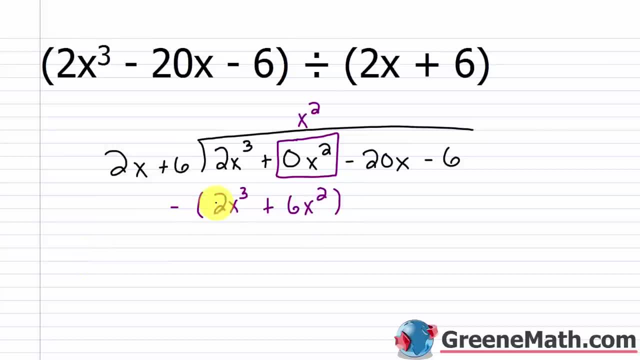 polynomials. I kind of got you to the point to where I didn't go through and do this extra step of putting parentheses around it, putting a minus in front and then erasing all this and changing the signs Again once you get comfortable. 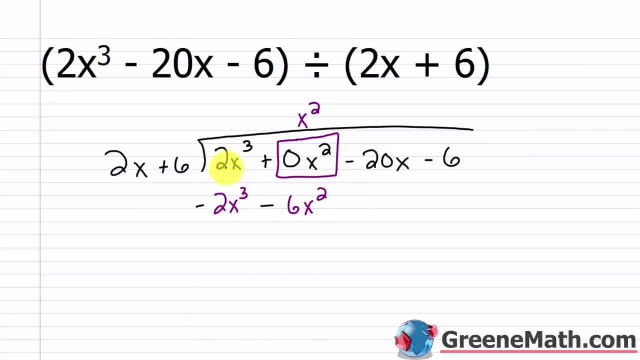 just change your signs and move on. Now I'm just going to add 2x cubed plus negative. 2x cubed is 0.. 0x squared minus. 6x squared is minus or negative. 6x squared. Scroll down and get a little room going. 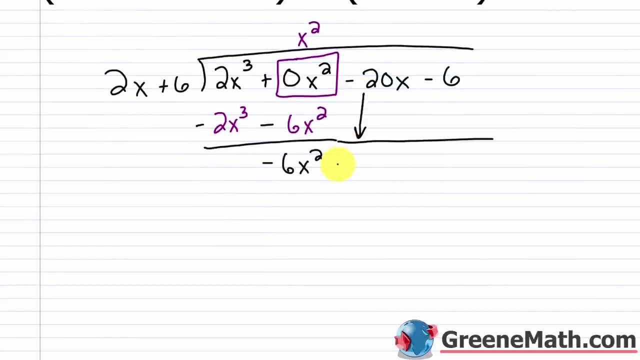 Now I'm going to bring down my next term, And my next term is a negative 20x. And then again I'm going to go leading term into leading term. So what is negative 6x squared over 2x? We know that this is going to. 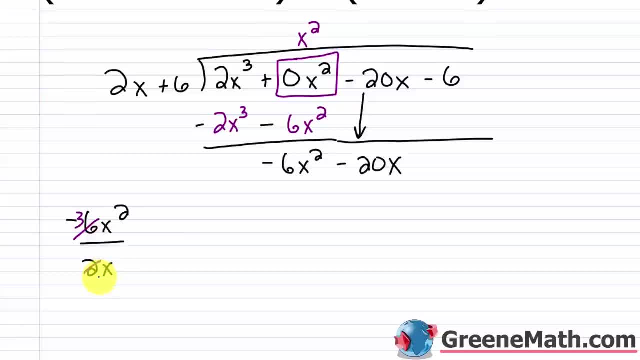 cancel with this and give me a negative 3. And x squared will cancel with x. That will give me x to the first power. So I'm going to have a minus 3x. I'm going to have a minus 3x. 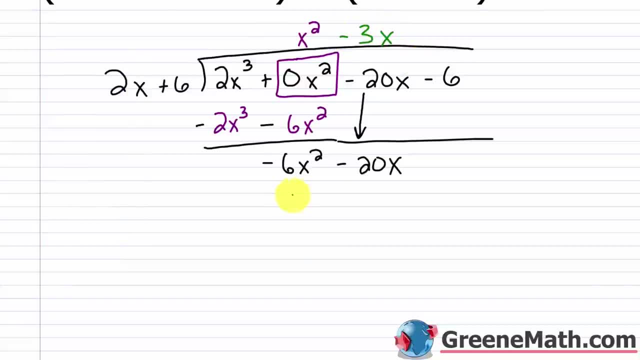 And I'm going to multiply: Negative 3x times 2x is negative 6x. squared Negative 3x times 6 is negative 18x. And again, I want to change the sign of each term here, Because I'm going to subtract this bottom one away. 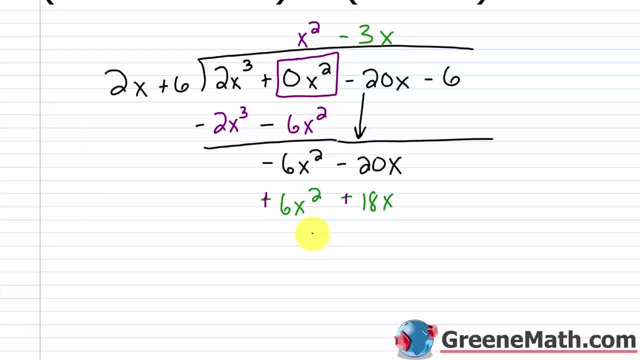 So this will be plus and this will be plus. So negative 6x squared plus 6x squared: that's going to cancel and be 0.. Negative 20x plus 18x: that's going to give me negative 2x. 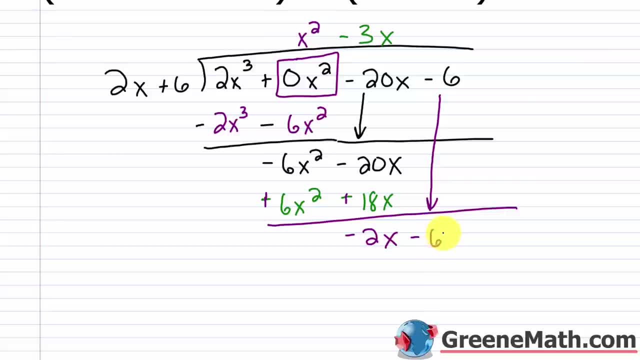 And then I'm going to bring down this last term here, which is negative 6.. And then my leading term, 2x, goes into negative 2x. how many times? So that's like saying negative 2x over 2x is what. 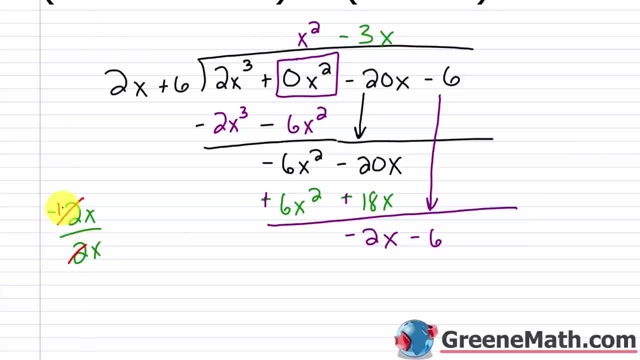 And we can all see that this is going to cancel with this and give me a negative 1.. And x over x is 1.. So this is going to end up being minus 1 here. So negative 1 times 2x is negative 2x. 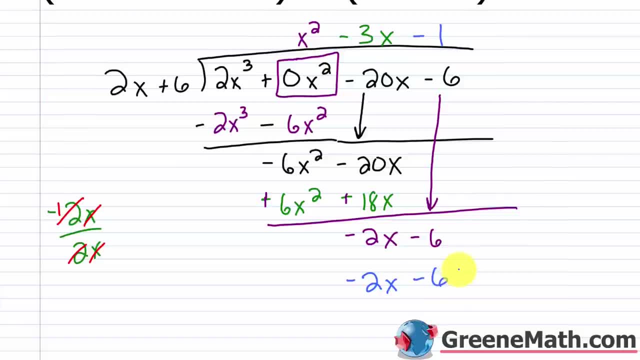 Negative 1 times 6 is minus 6.. If I subtract the same thing away from itself, I get 0.. So this will become plus. This will become plus Negative: 2x plus 2x is 0.. Negative: 6 plus 6 is 0. 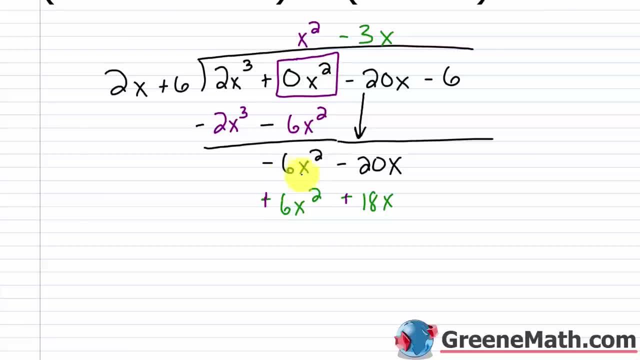 So this will be plus and this will be plus. So negative 6x squared plus 6x squared, that's going to cancel and be 0. 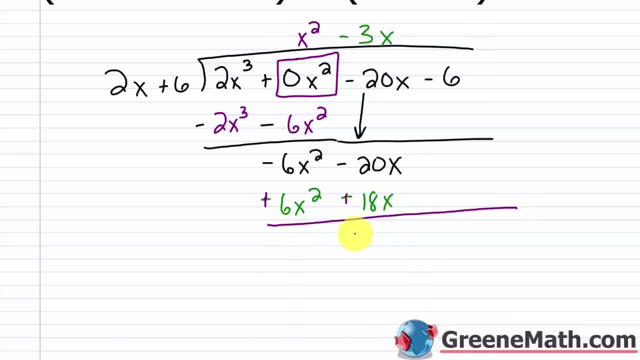 Negative 20x plus 18x, that's going to give me negative 2x. And then I'm going to bring down this last term here, which is negative 6. 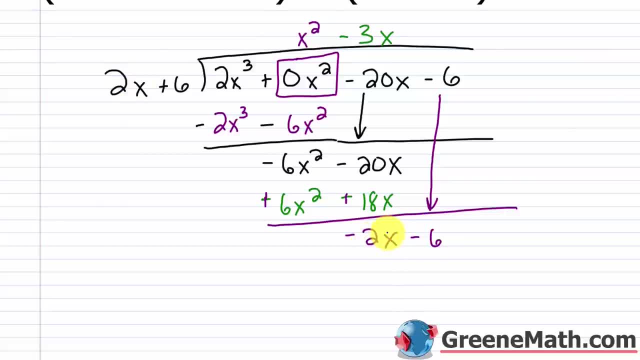 And then my leading term, 2x, goes into negative. Negative 2x, how many times? 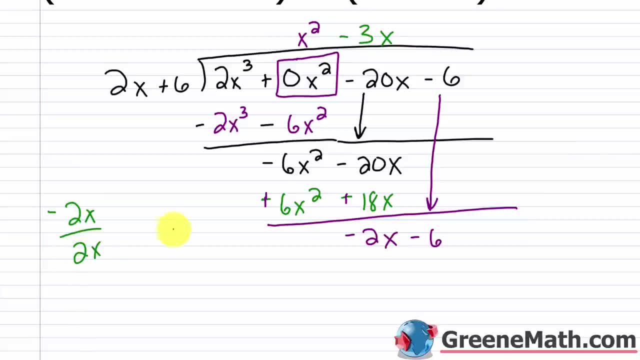 So that's like saying negative 2x over 2x is what? And we can all see that this is going to cancel with this and give me a negative 1. And x over x is 1. So this is going to end up being minus 1 here. So negative 1 times 2x is negative 2x. Negative 1 times 6 is minus 6. 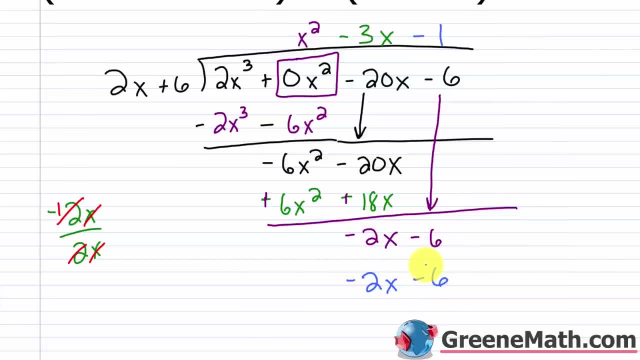 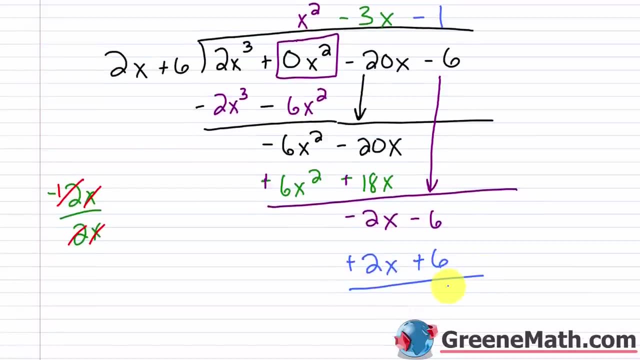 If I subtract the same thing away from itself, I get 0. This will become plus. This will become plus. Negative 2x plus 2x is 0. Negative 6 plus 6 is 0. So there's no remainder. 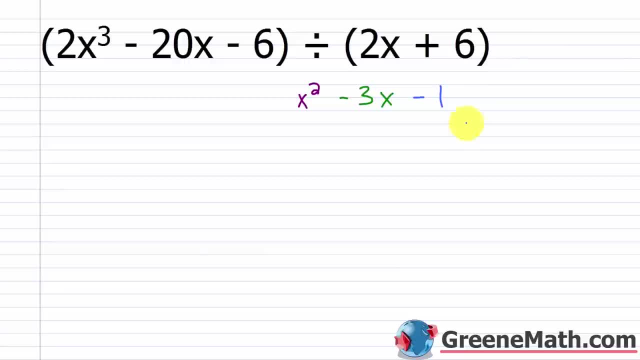 So I get x squared minus 3x minus 1. All right, so remember, I like to check things. 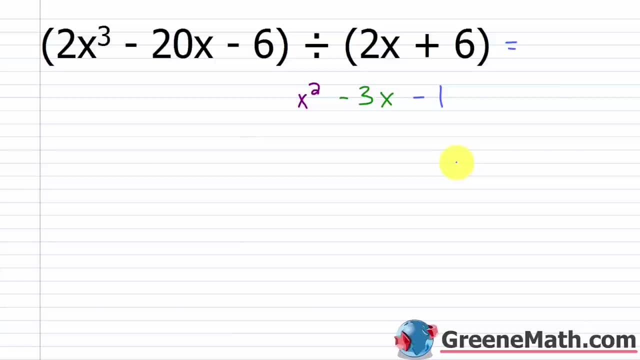 And if you don't like to check things, just skip ahead in the video. It's no problem. 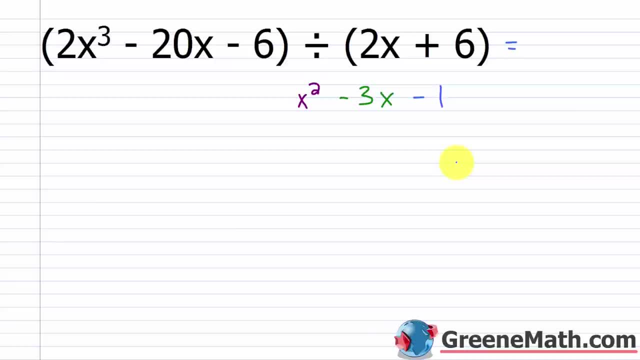 It usually takes about two, three minutes to check something. And I understand that you're going to get on timed examinations where you just can't check it. But particularly when you're doing homework and your teacher's grading it, you want to check it and make sure you got the right answer. You don't want to blow a problem, right? So let's go ahead and just multiply. This guy right here. This guy right here. Times this guy right here. 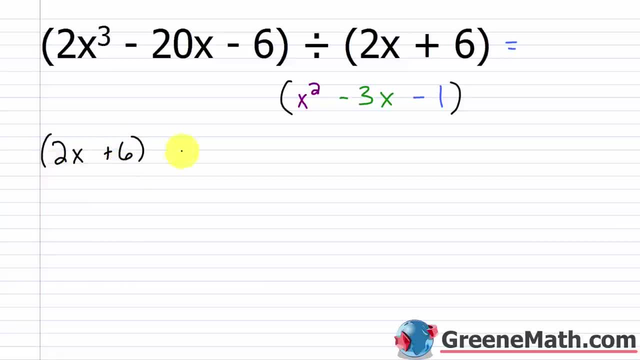 So I'll have 2x plus 6. That's multiplied by x squared minus 3x minus 1. So 2x times x squared is 2x cubed. 2x times negative 3x is minus 6x squared. 2x times negative 1 is minus 2x. 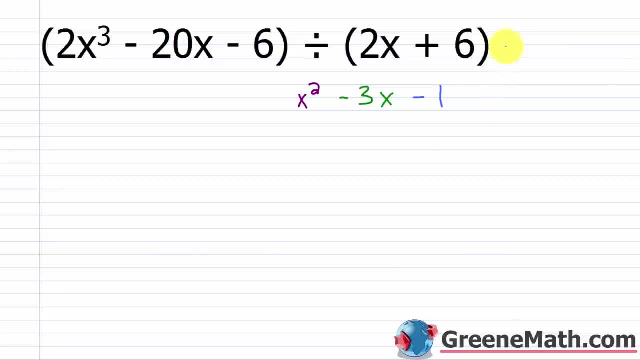 So there's no remainder. So I get x squared minus 3x minus 1.. Alright, so remember, I like to check things, And if you don't like to check things, just skip ahead in the video, It's no problem. It usually takes about 2-3 minutes to check something. 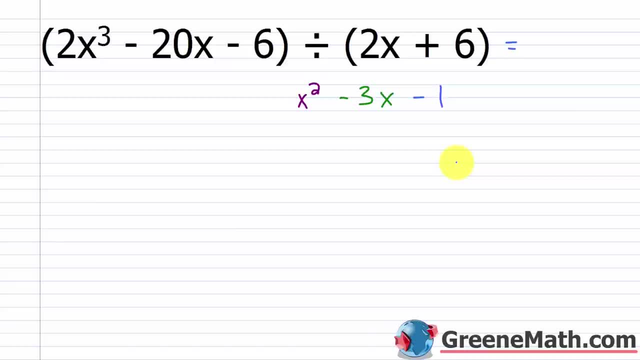 And I understand that you're going to get on timed examinations where you just can't check it. But particularly when you're doing homework and your teacher is grading it, you want to check it and make sure you got the right answer. You don't want to blow a problem. 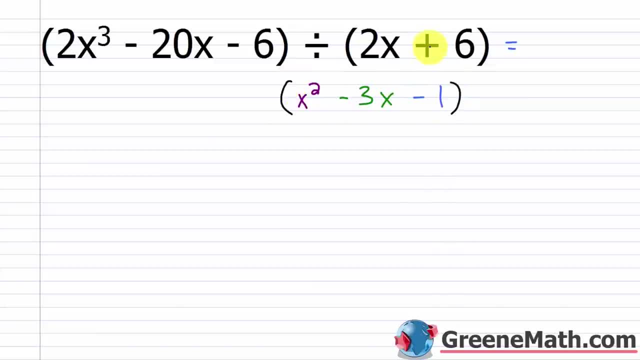 So let's go ahead and just multiply this guy right here times this guy right here, Your quotient by your divisor should give your dividend back. So I'll have 2x plus 6, that's multiplied by x squared minus 3x minus 1.. 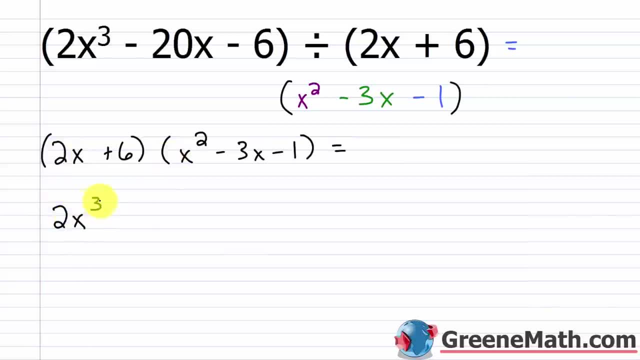 So 2x times x squared is 2x cubed. 2x times negative, 3x is minus 6x squared. 2x times negative, 1 is minus 2x. 6 times x squared is plus 6x squared. 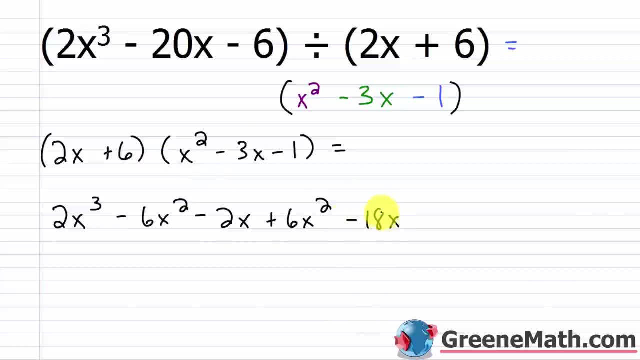 6 times negative, 3x is minus 18x, And then 6 times negative, 1 is minus 6.. So if I combine like terms here, I've got like terms here, I've got like terms here- I'd have 2x cubed. 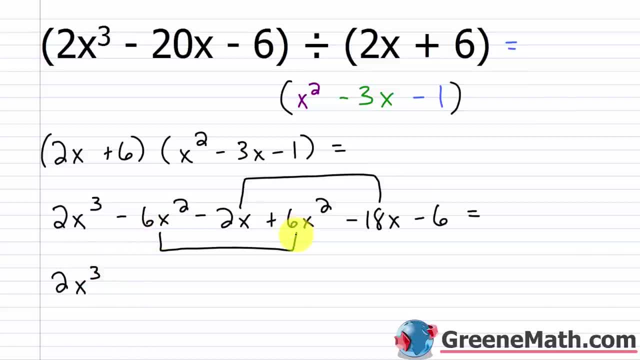 negative: 6x squared plus 6x squared is 0x squared, So I don't have to write that, So I can put plus 0x squared, kind of like I did when I set up the division, or I don't have to put it. 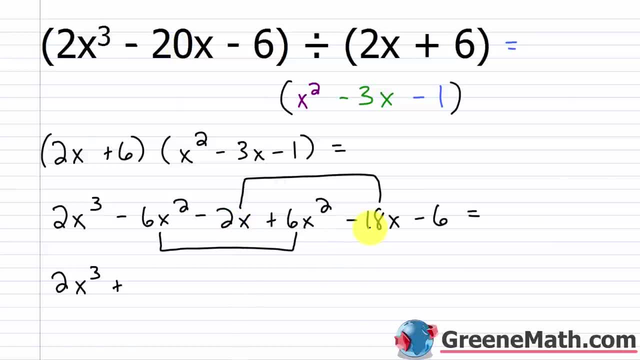 Then I have negative 2x minus 18x, that's negative 20x, and then lastly, minus 6. And that completely matches this right here: 2x cubed minus 20x minus 6. so we know we have the correct answer. 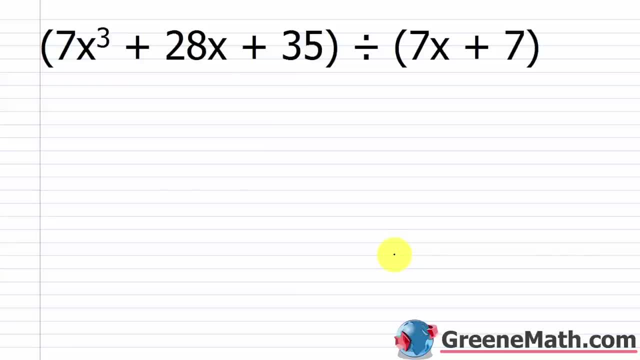 Alright, let's take a look at it all. We have 7x cubed plus 28x, plus 35, and this is divided by 7x plus 7.. So again, let's take this guy right. here we have 7x cubed. 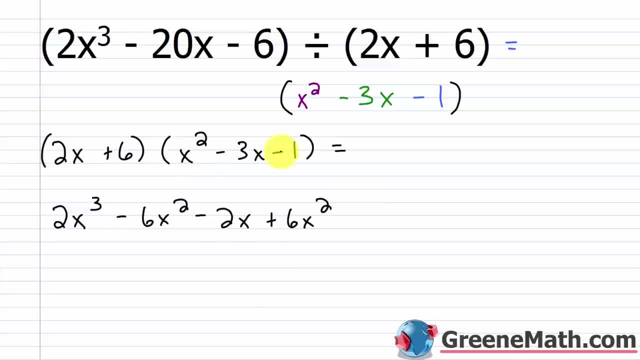 6 times x squared is plus 6x squared. 6 times negative 3x is minus 8x squared. 6 times negative 3x is minus 18x. And then 6 times negative 1 is minus 6. 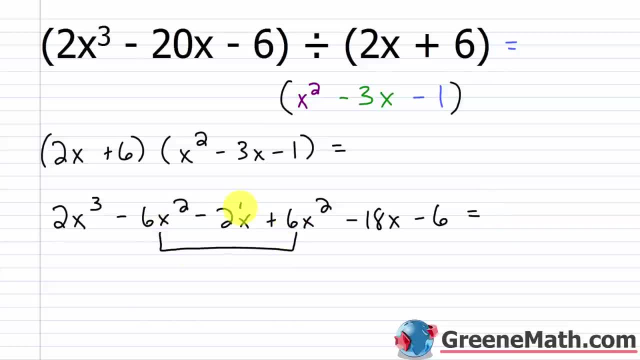 So if I combine like terms here, I've got like terms here. I've got like terms here. I'd have 2x cubed. 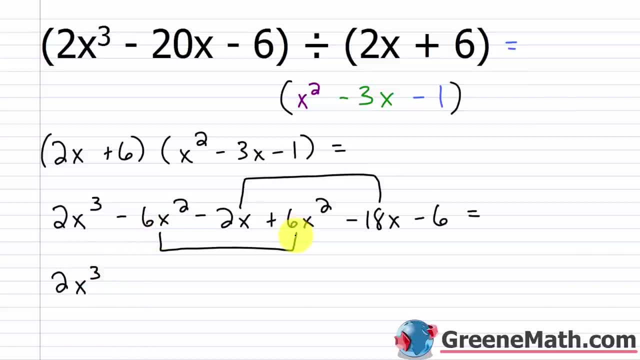 Negative 6x squared plus 6x squared is 0x squared, right? So I don't have to write that. 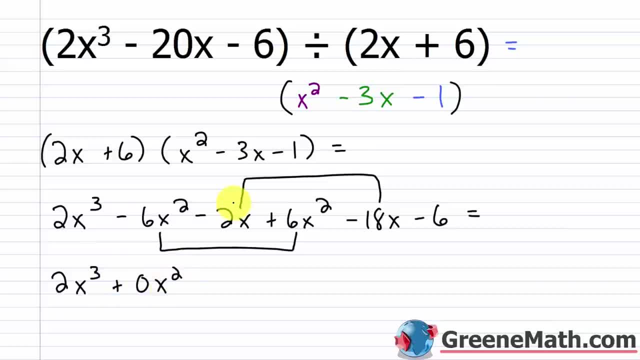 So I could put plus 0x squared, kind of like I did when I set up the division, or I don't have to put it, right? I can leave it just like it's going to be up here. 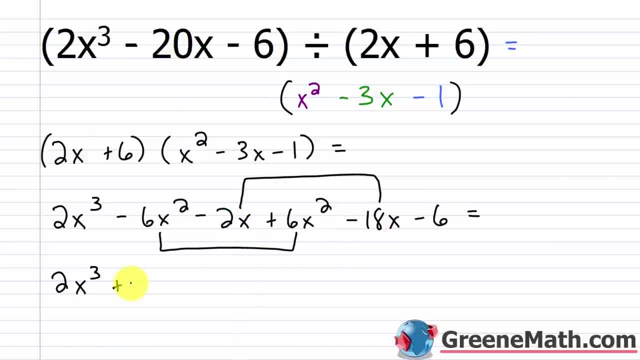 Then I have negative 2x minus 18x. That's negative 20x. 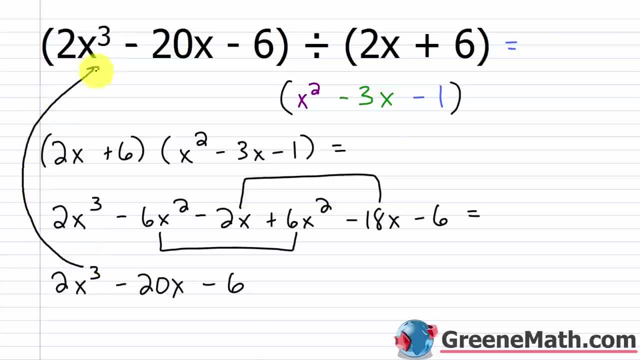 And then lastly, minus 6. And that completely matches this right here. 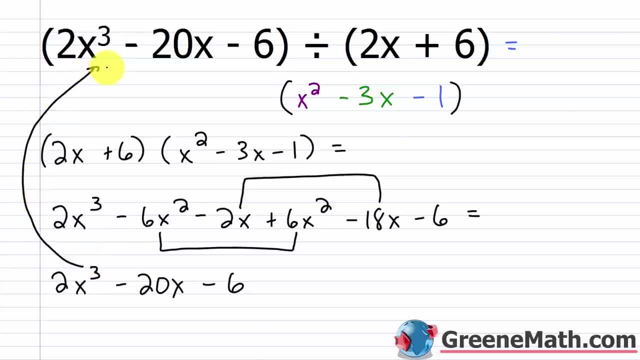 2x cubed minus 20x minus 6. So we know we have the correct answer. 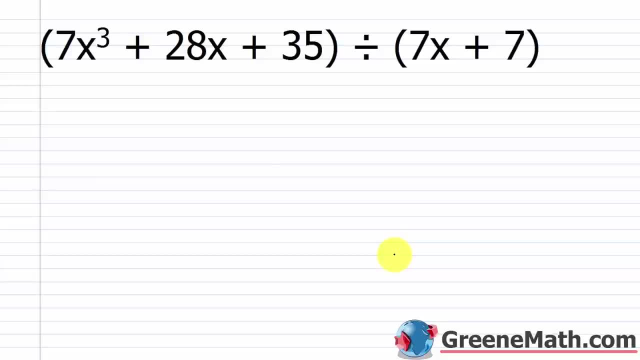 All right, let's take a look at it all. We have 7x cubed plus 28x plus 35. 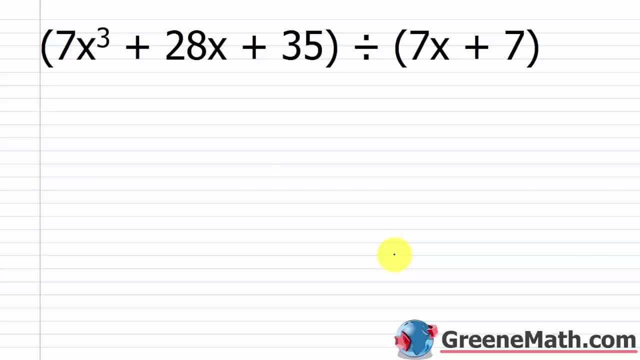 And this is divided by 7x plus 7. So again, let's take this guy right here. We have 7x cubed. Now, the next one is 28x. This is to the first power here. So I'm missing my x squared term again. So plus 0x squared. 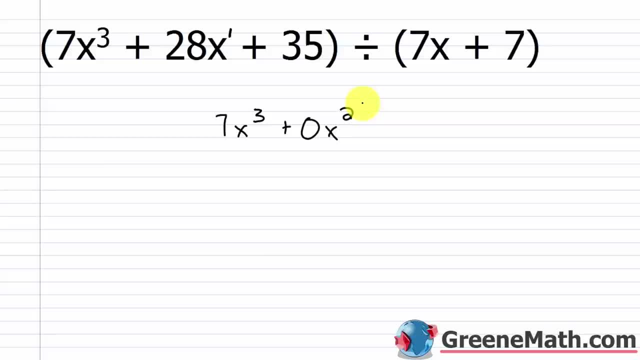 Again, if you're missing something, just write the coefficient as 0, and then give yourself a representation of the variable raised to that missing power. 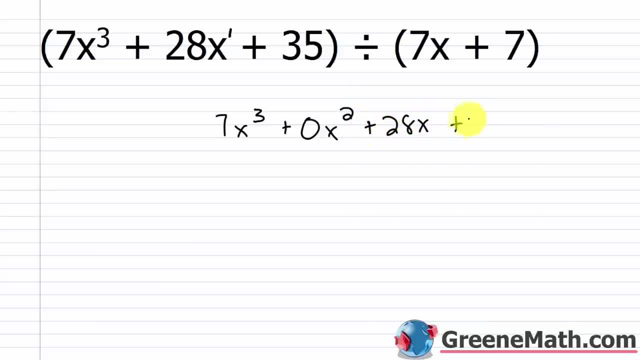 Then plus 28x, then plus 35. 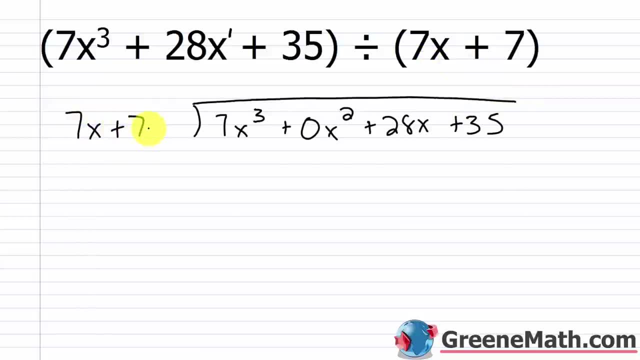 Then this guy over here, 7x plus 7. That's going to go off to the side. 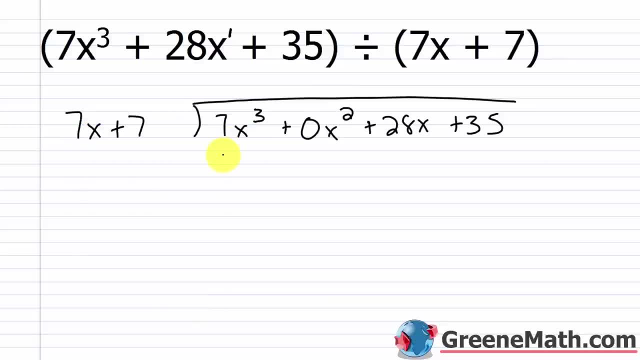 And then we divide like we normally do. Leading term into leading terms. So 7x cubed over 7x. This is going to cancel with this. And give me a 1. 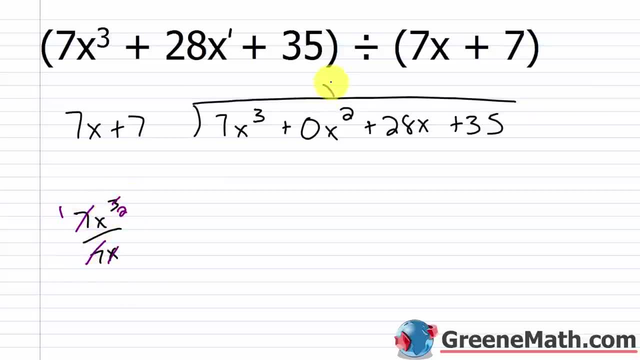 x cubed over x is x squared. So that's going to go right here. And then I'm going to multiply. 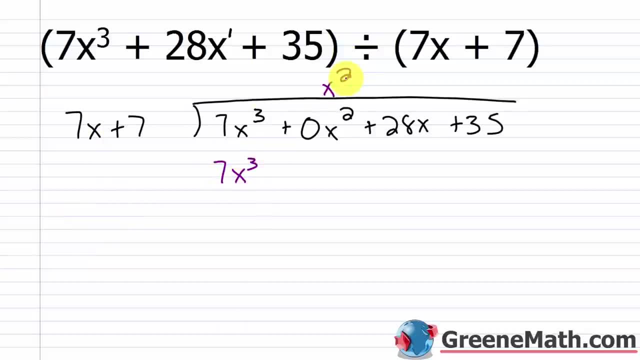 x squared times 7x is 7x cubed. x squared times 7 is plus 7x squared. So I'm going to change the sign of each term here now. This is going to become minus. 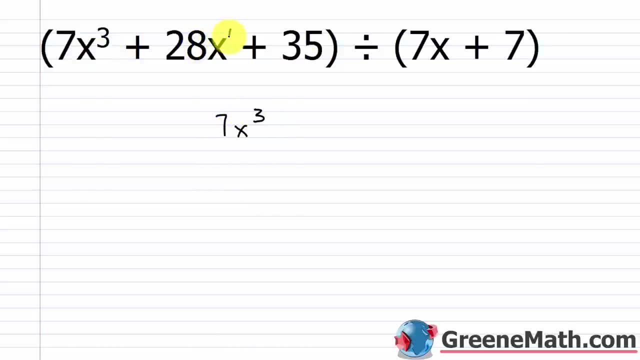 now the next one is 28x. this is to the first power here. so I'm missing my x squared term again. so plus 0x squared Again. if you're missing something, just write the coefficient as 0 and then give yourself a representation of the variable. 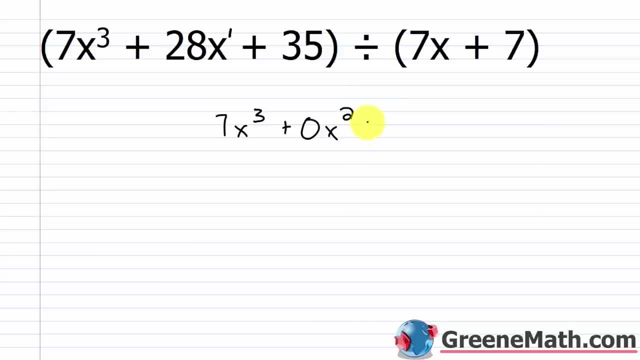 raised to that missing power. Then plus 28x, then plus 35. Then this guy over here, 7x plus 7. that's going to go off to the side. and then we divide, like we normally do, Leading term into leading term. so 7x cubed. 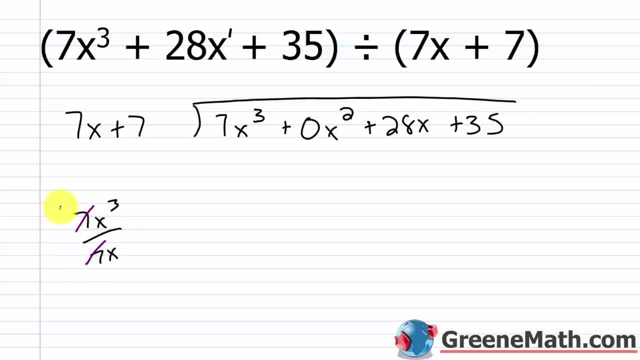 over 7x. this is going to cancel with this and give me a 1 x cubed over x is x squared. So that's going to go right here, and then I'm going to multiply x squared times: 7x is 7x cubed. 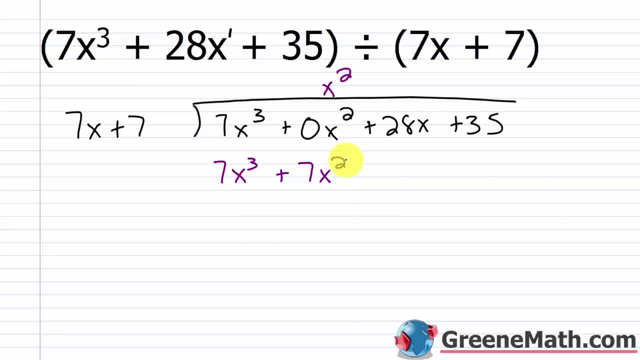 x squared times 7 is plus 7x squared, So I'm going to change the sign of each term here now. This is going to become minus. this is going to become minus and I'm going to add 7x cubed plus negative. 7x cubed is 0. 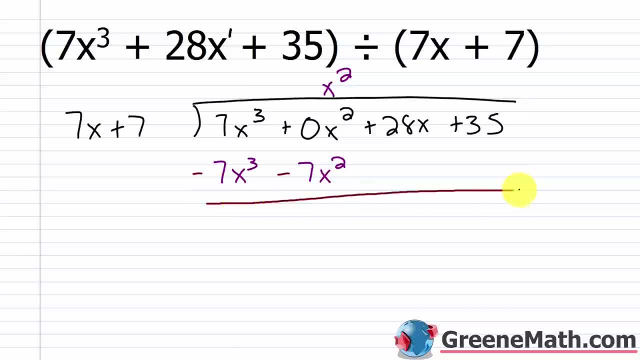 0x squared. minus 7x squared is negative 7x squared. Let's bring down the next term, which is plus 28x, and then let's go leading term into leading term. So I have negative 7x squared over 7x and I'm 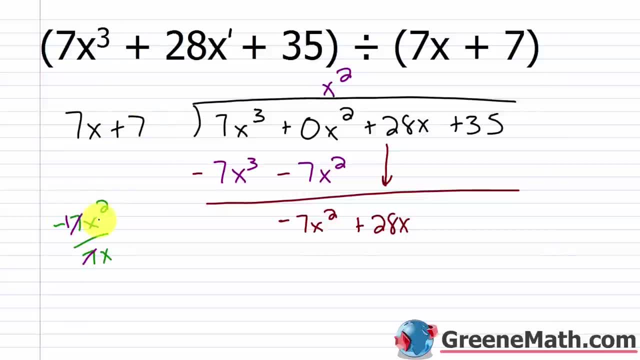 going to cancel this with this. That's going to give me negative 1 and then x squared over x. This is going to cancel with this and give me x to the first power. So this is going to be negative x to the first power. 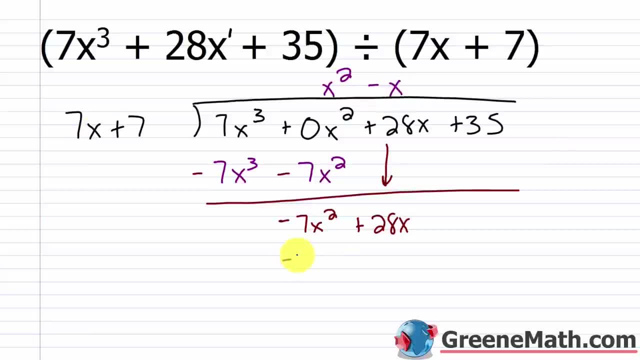 and then I want to multiply: Negative x times 7x is going to be negative 7x squared, Negative x times 7 is minus 7x, And again change the sign of each term here. So this has become plus and this has become plus. 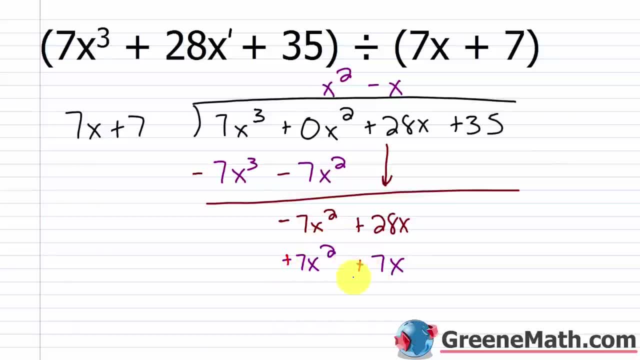 So negative. 7x squared plus 7x squared is 0.. 28x plus 7x is 35x. So this is 35x, and then this comes down: This is plus 35. Then 7x goes into 35x. This is going to become minus. 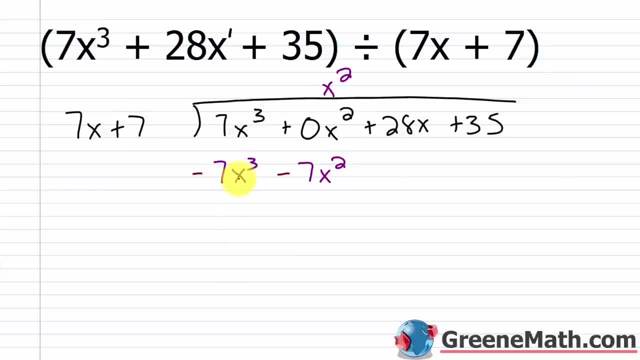 And I'm going to add 7x cubed plus negative 7x cubed is 0. 0x squared minus 7x squared is negative 7x squared. Let's bring down the next term, which is plus 28x. And then let's go leading term into leading term. So I have negative 7x squared over 7x. And I'm going to cancel this with this. That's going to give me a negative 1. And then x squared over x. This is going to cancel with this and give me x to the first power. 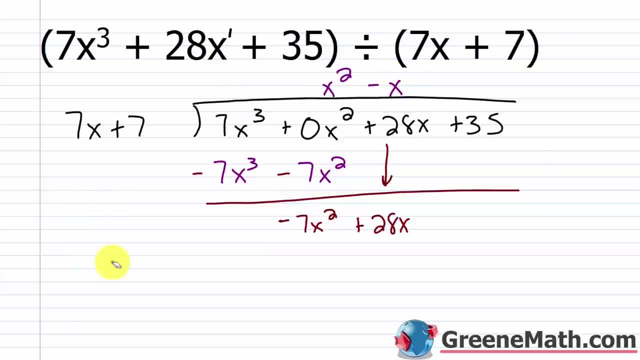 So this is going to be negative x to the first power. And then I want to multiply. Negative x times 7x is going to be negative 7x squared. Negative x times 7 is minus 7x. 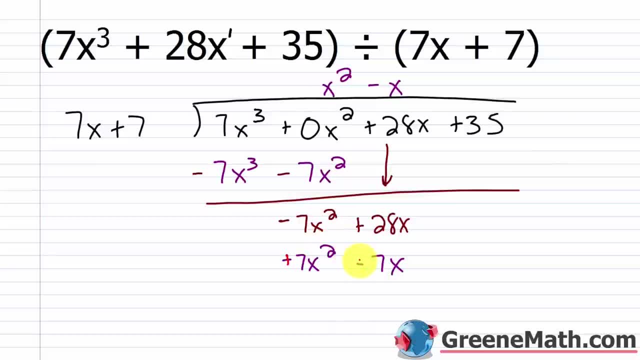 And again, change the sign of each term here. So this has become plus and this has become plus. 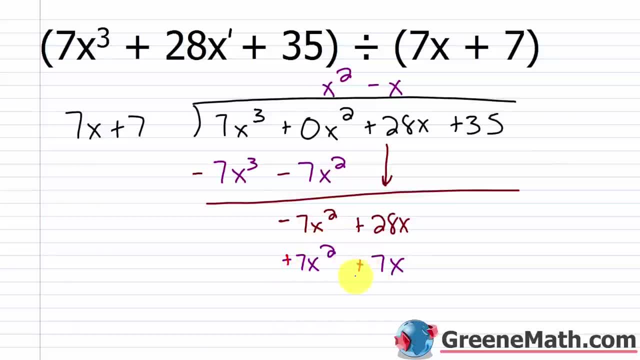 So negative 7x squared plus 7x squared is 0. 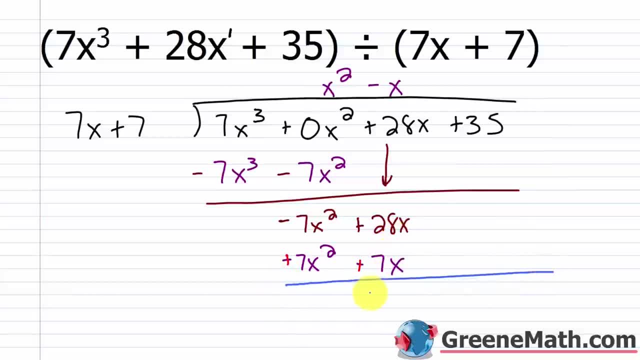 28x plus 7x is 35x. So this is 35x. 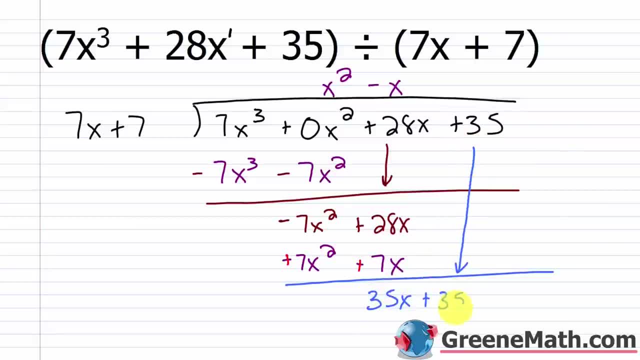 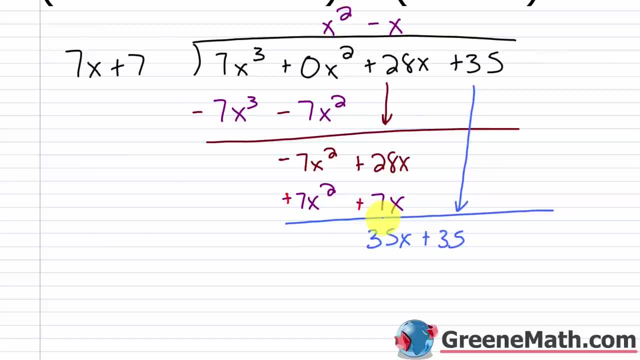 And then this comes down. This is plus 35. Then 7x goes into 35x. 5x, 5 times. We can all see that 35 would cancel with 7 and give me a 5. x over x is 1. So this is going to be plus 5. 5 times 7x is 35x. 5 times 7 is 35. 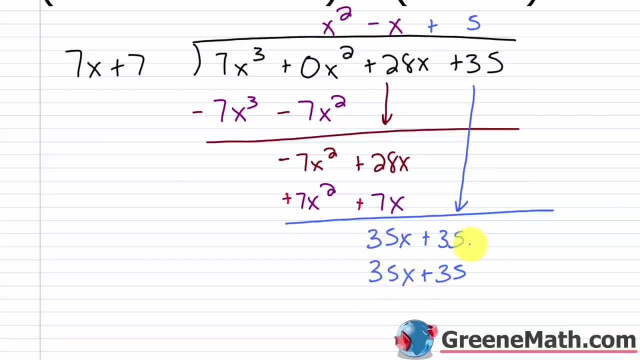 If I subtract 35x plus 35 from that, I'm going to get 0. This would become negative. 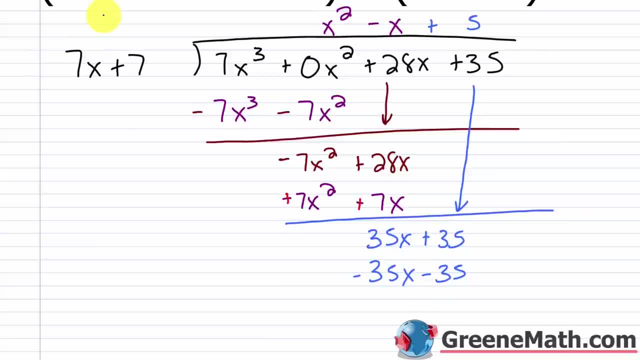 And so with this. So 35x plus negative 35x is 0. 35 minus 35 is 0. So there's no remainder. 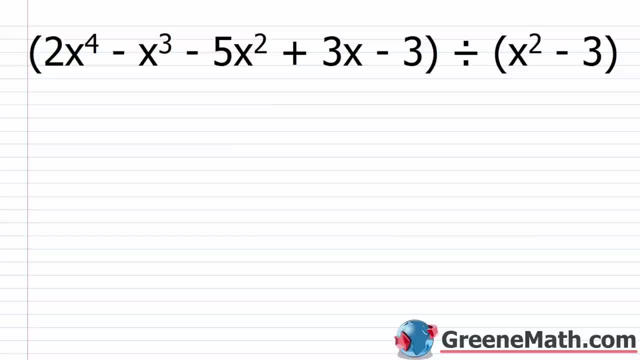 So we get x squared minus x plus 5. All right, let's do one final problem. 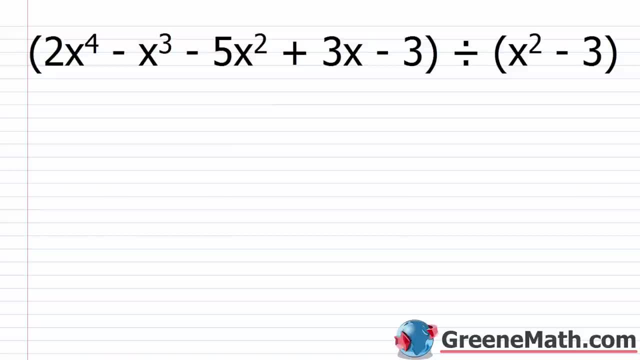 The only difference here is I'm going to put the missing term in the divisor instead of the dividend. 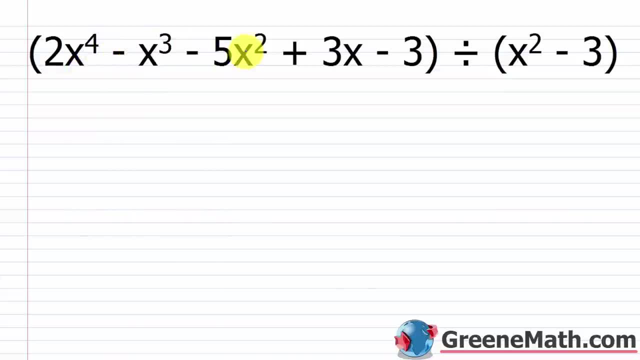 So I have 2x to the fourth power minus x cubed minus 5x squared plus 3x minus 3. So let's set this up. 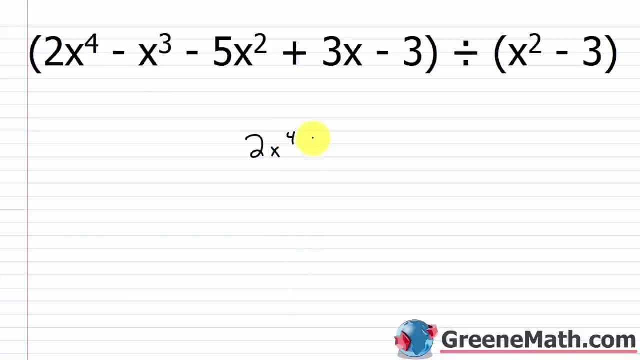 My dividend is 2x to the fourth power minus x cubed minus 5x squared. Plus 3x. 3x minus 3. 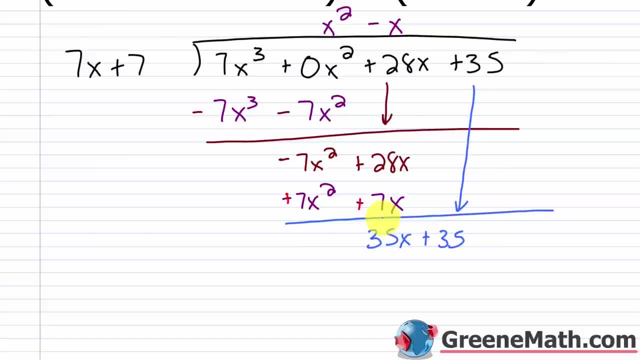 five times. We can all see that 35 would cancel with 7 and give me a 5.. x over x is 1.. So this is going to be plus 5.. 5 times 7x is 35x 5 times. 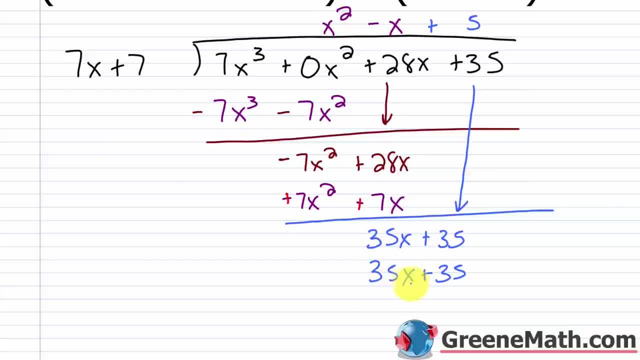 7 is 35. If I subtract 35x plus 35 from that, I'm going to get 0. This would become negative, and so this. So 35x plus negative 35x is 0.. 35 minus 35. 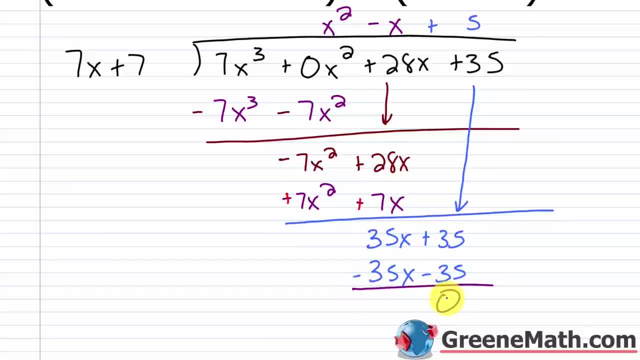 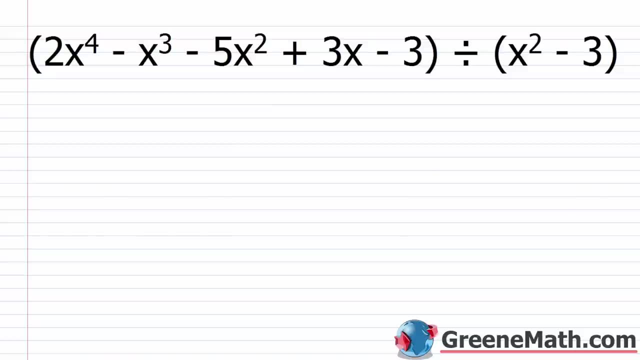 is 0.. So there's no remainder here. So we get x squared minus x plus 5.. Alright, let's do one final problem. The only difference here is I'm going to put the missing term in the divisor instead of the dividend, So I have 2x. 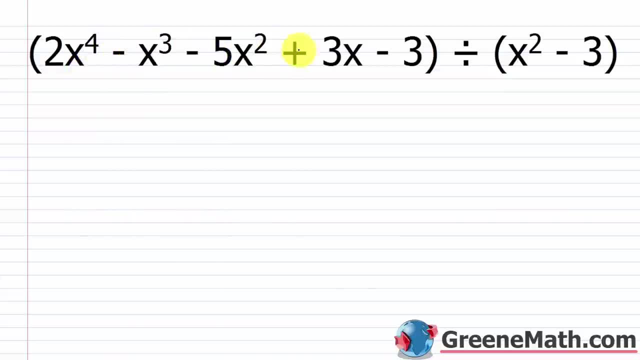 to the fourth power minus x cubed minus 5x, squared plus 3x minus 3.. We're dividing by x squared minus 3.. So let's set this up: My dividend is 2x to the fourth power minus x cubed minus 5x. 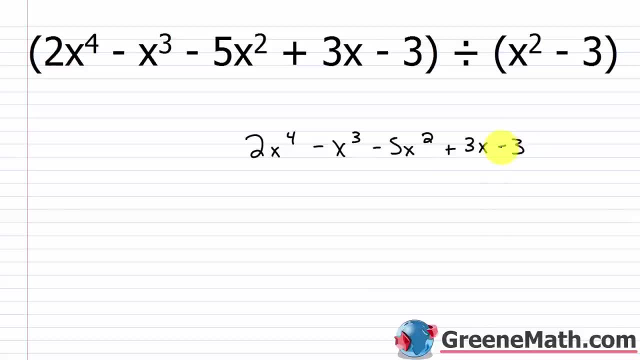 squared plus 3x minus 3.. Then over here my divisor is x squared minus 3.. So x squared, I'm missing my x to the first power. So I'm going to put plus 0x and then I have minus 3.. 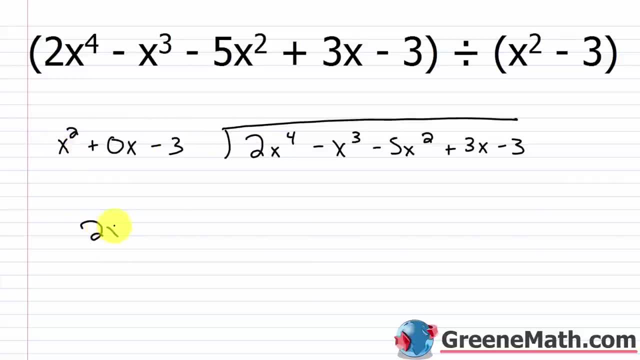 So again, leading term into leading term. So what is 2x to the fourth power over x squared? Well, we know that this is going to cancel with this and give me 2x squared. Alright, this would cancel out. So 2x squared. 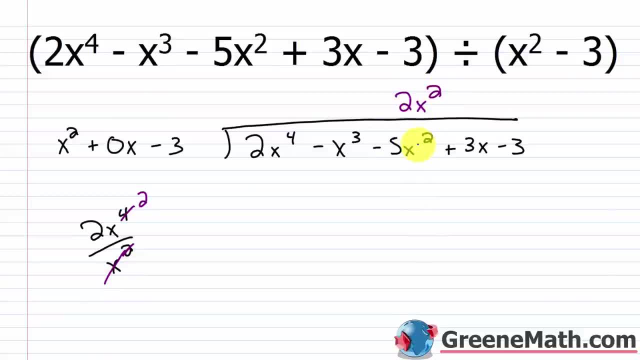 Again, I'm going to write that over the term that has x squared in it, And then I'm going to multiply: 2x squared times x squared is 2x to the fourth power: 2x squared times 0x is 0x. 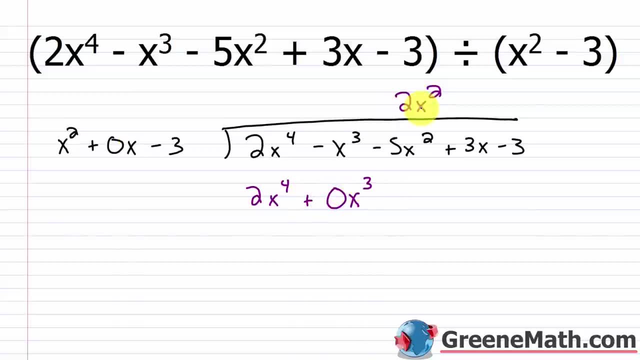 cubed, Then 2x squared times negative 3 is minus 6x squared. So we're subtracting this guy away. So that means I'm going to change this to a minus. I'm going to change this to a minus. 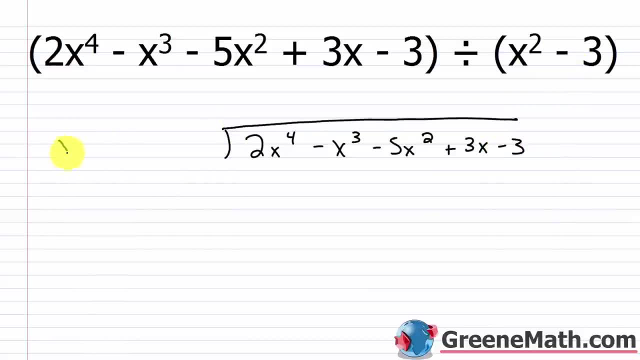 Then over here, my divisor is x squared minus 3. So x squared. I'm missing my x to the first power. 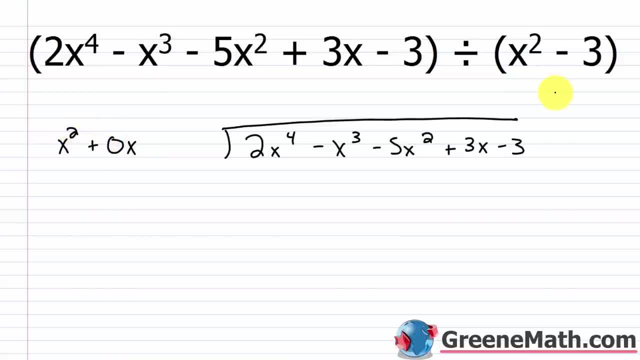 So I'm going to put plus 0x. And then I have minus 3. 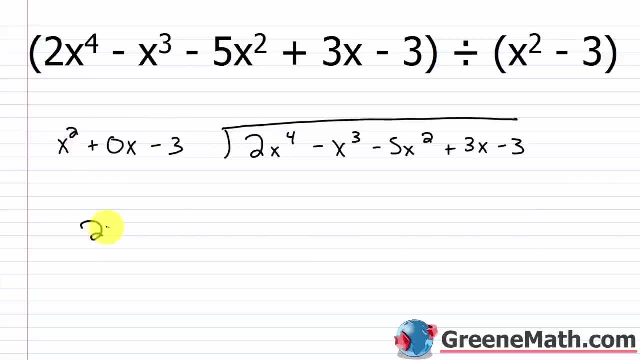 So again, leading term into leading term. So what is 2x to the fourth power over x squared? 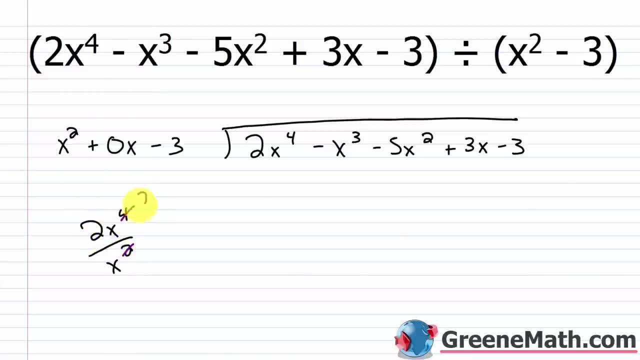 Well, we know that this is going to cancel with this and give me 2x squared. This would cancel out. So 2x squared. 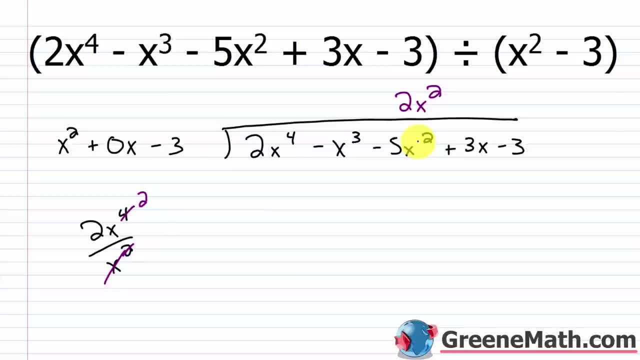 Again, I'm going to write that over the term that has x squared in it. And then I'm going to multiply. 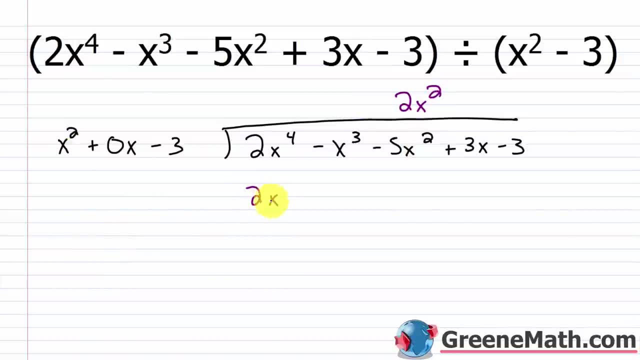 2x squared times x squared is 2x to the fourth power. 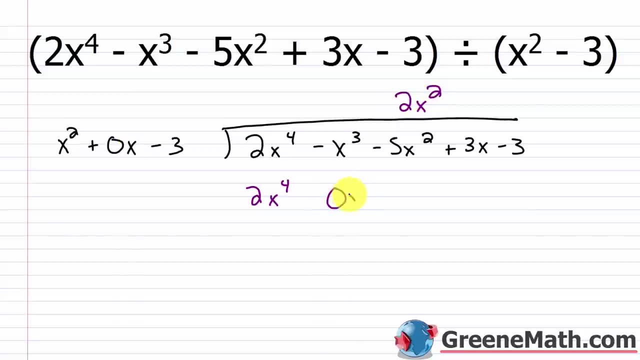 2x squared times 0x is 0x cubed. 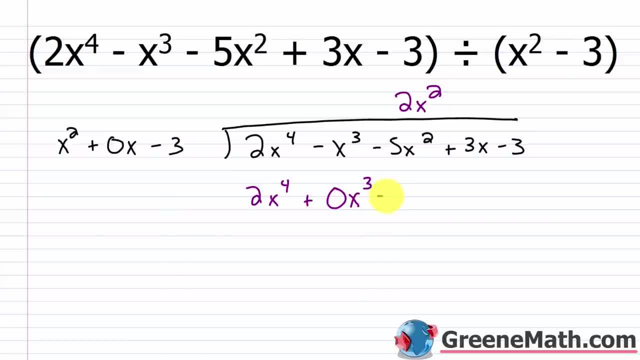 Then 2x squared times negative 3 is minus 6x squared. 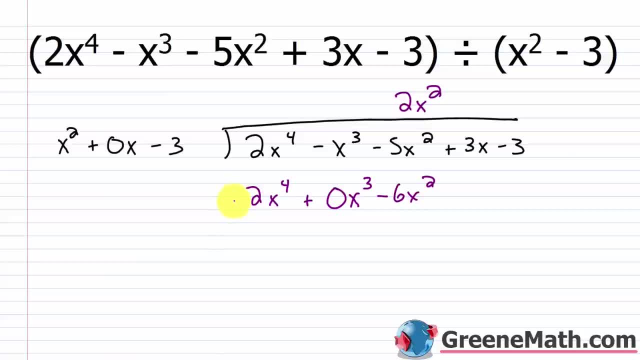 So we're subtracting this guy away. So that means I'm going to change this to a minus. I'm going to change this to a minus. And I'm going to change this to a plus. So let's go ahead and add. 2x to the fourth power minus 2x to the fourth power is 0. 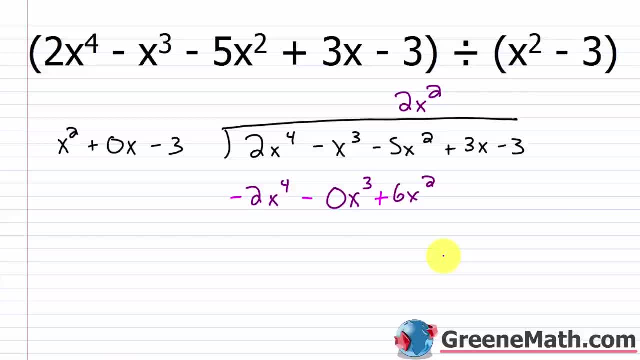 Negative x cubed minus 0x cubed is negative x cubed. 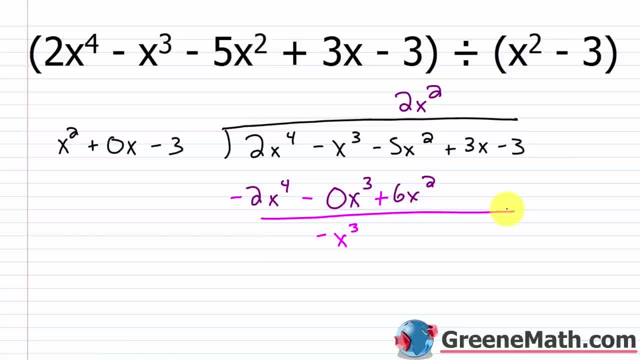 Then negative 5x squared plus 6x squared is 1x squared or just x squared. All right. 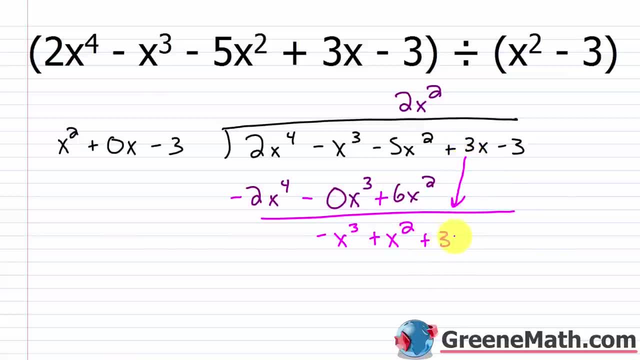 So now I'm just going to bring down this 3x. And I'm going to go. Leading term into leading term. 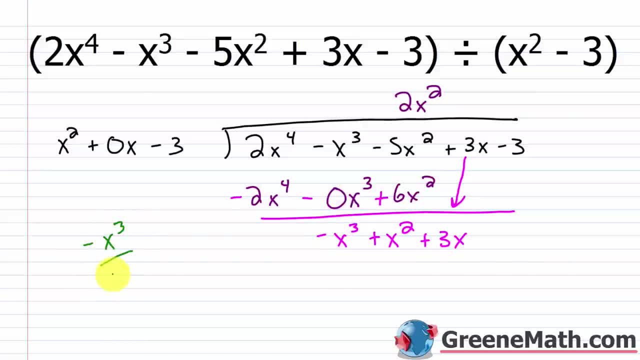 So what is negative x cubed over x squared? Well, we know that this is going to cancel out with two factors of x from that numerator. So this would be negative x to the first power. So minus x. And then we're going to multiply. Negative x times x squared is negative x cubed. 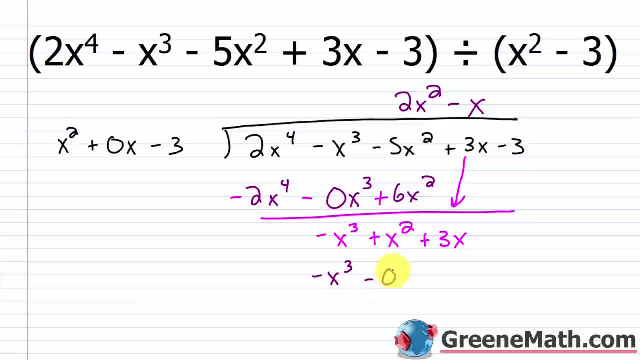 Negative x times 0x is minus 0x squared. 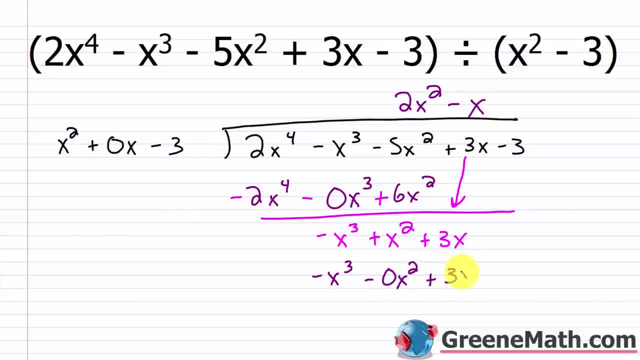 Negative x times negative 3. 3 is positive 3x. 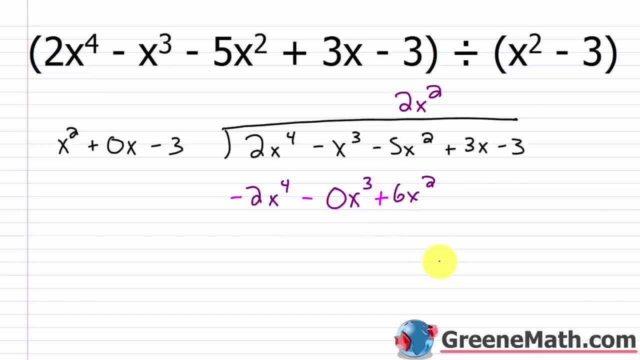 And I'm going to change this to a plus. So let's go ahead and add 2x to the fourth power. minus 2x to the fourth power is 0.. Negative x cubed minus 0x cubed is negative x cubed. 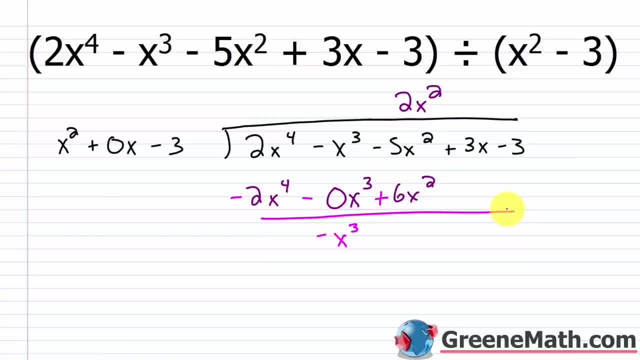 Then negative: 5x squared plus 6x squared is 1x squared or just x squared. Alright, so now I'm just going to bring down this 3x And I'm going to go leading term into leading term. So what is? 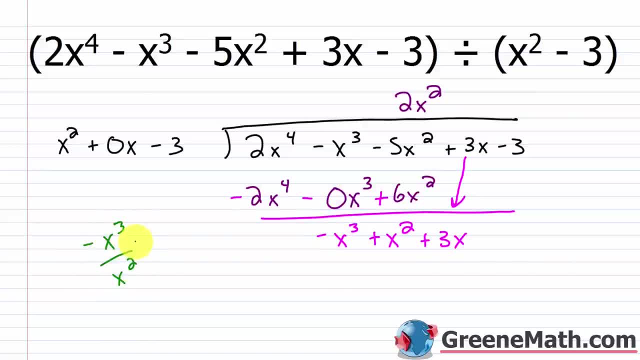 negative x cubed over x squared. Well, we know that this is going to cancel out with two factors of x from that numerator. So this would be negative x to the first power, So minus x. And then we're going to multiply Negative x times x squared is negative x. 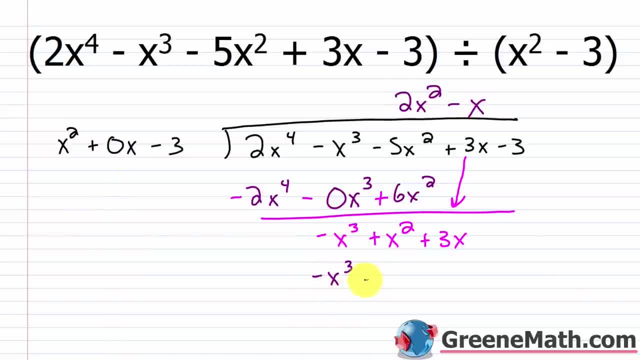 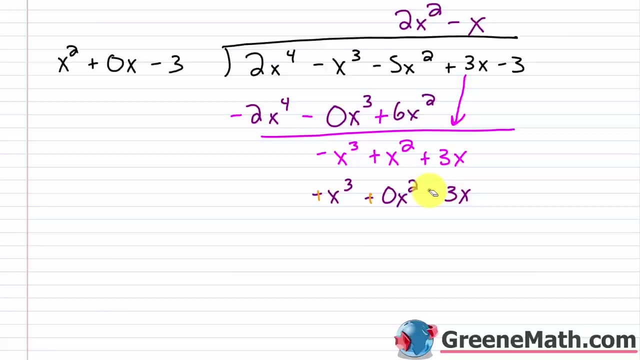 cubed: Negative x times 0x is minus 0x. squared Negative x times negative: 3 is positive 3x. So let me change the signs here. So this would be positive, positive, and then this guy is going to be negative. 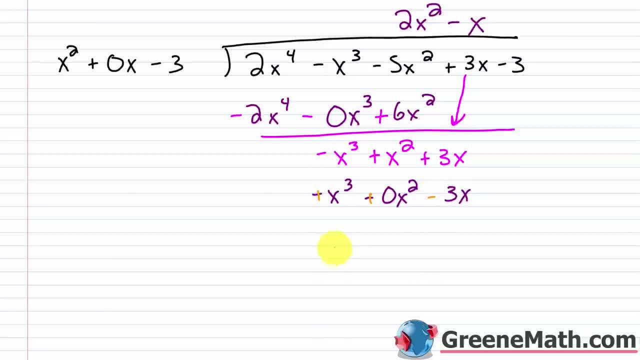 So negative x cubed plus x cubed is 0.. x squared plus 0x squared is just x squared. So then 3x minus 3x we could put plus 0x And then we can bring down this negative 3.. 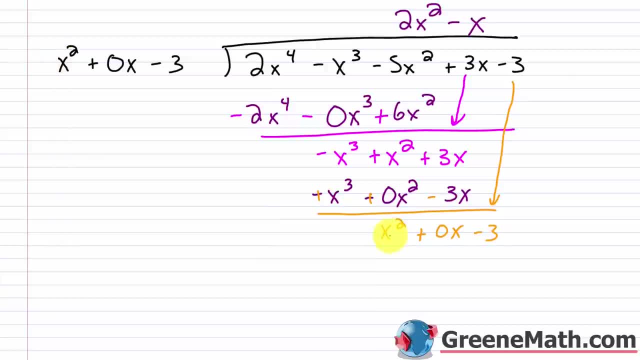 And now, once again, I'm going to do leading term into leading term: x squared over x squared is 1.. So I'm going to put plus 1 here And I'm going to multiply 1 times. x squared is x squared. 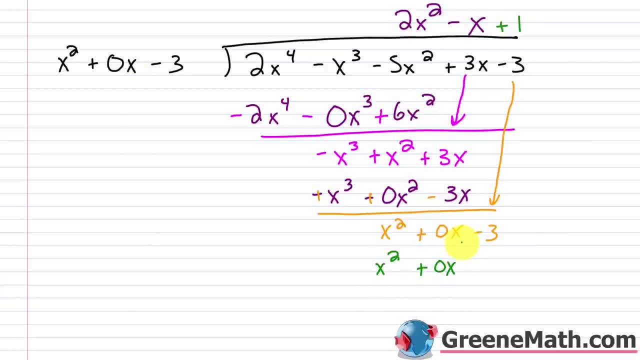 1 times 0x is 0x, And then 1 times negative, 3 is minus 3.. So I have the same thing over itself. If I'm going to subtract here, If I subtract the same thing away from itself, I get 0. 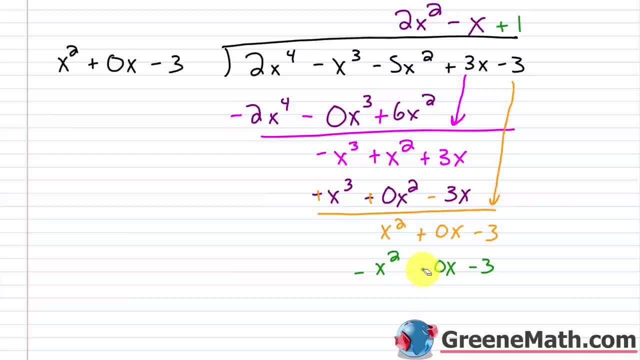 x squared minus x squared is 0.. 0x minus 0x is 0.. Negative 3 plus 3 is 0.. So this becomes 0.. So 2x squared minus x plus 1 is our answer. Hello and welcome to. 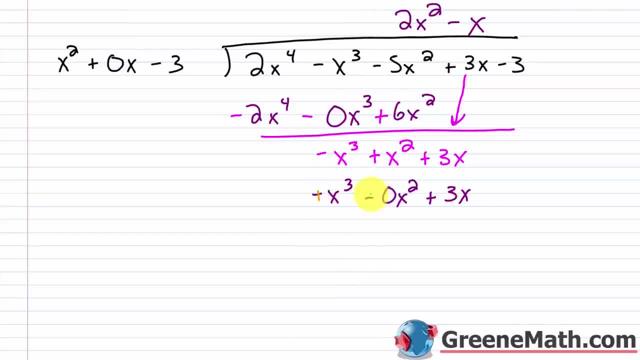 So let me change the signs here. So this will be positive, positive. And then this guy is going to be negative. 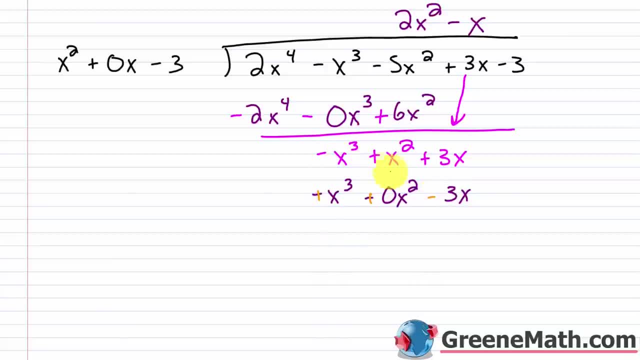 So negative x cubed plus x cubed is 0. x squared plus 0x squared is just x squared. 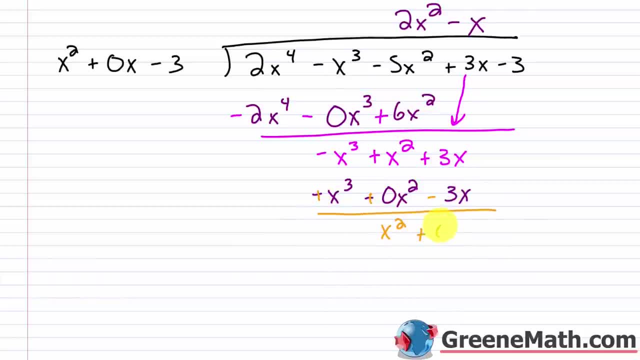 So then 3x minus 3x, we could put plus 0x. And then we can bring down this negative 3. 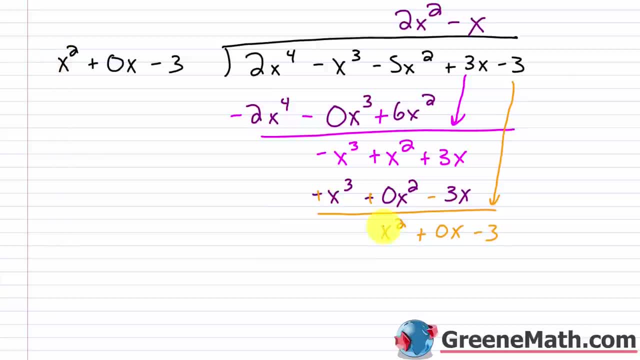 And now once again, I'm going to do. Leading term into leading term. x squared over x squared is 1. So then I'm going to put plus 1 here. And I'm going to multiply. 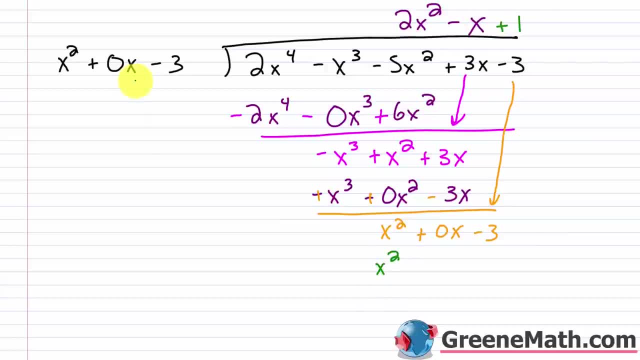 1 times x squared is x squared. 1 times 0x is 0x. And then 1 times negative 3 is minus 3. So I have the same thing over itself. If I'm going to subtract here, if I subtract the same thing away from itself, I get 0. x squared minus x squared is 0. 0x minus 0x is 0. Negative 3 plus 3 is 0. So this becomes 0. 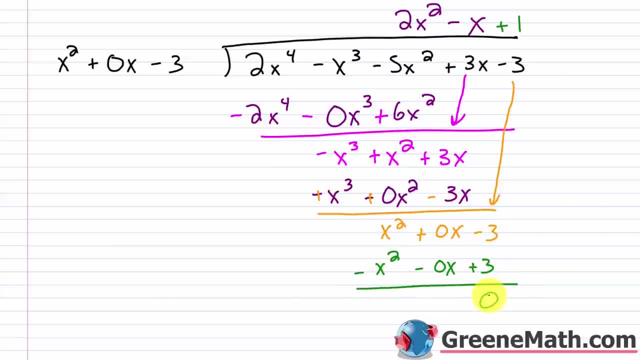 So 2x squared minus x plus 1 is our answer. 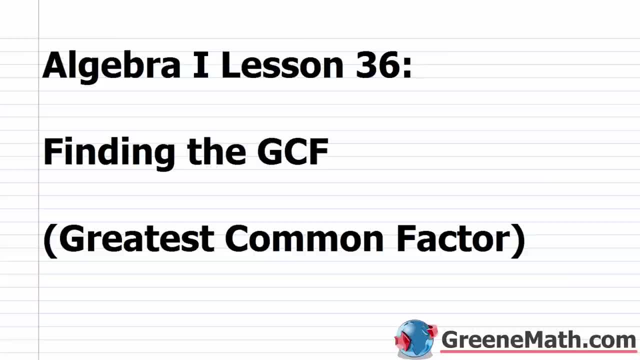 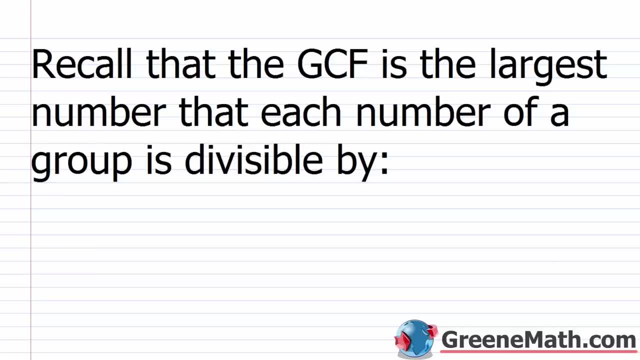 Hello and welcome to Algebra 1, Lesson 36. In this video, we're going to learn about finding the GCF, otherwise known as the greatest common factor. So hopefully you learned how to find the greatest common factor in pre-algebra. If this is new to you, I'm going to do enough of a review here to where you can catch on very quickly. So I want you to recall that the GCF, again, that's the greatest common factor, or some people like to say the greatest common divisor. This is the largest number that each number of a group is divisible by. So let me give you a quick example. Let's say you had two numbers, let's say 12 and 18. 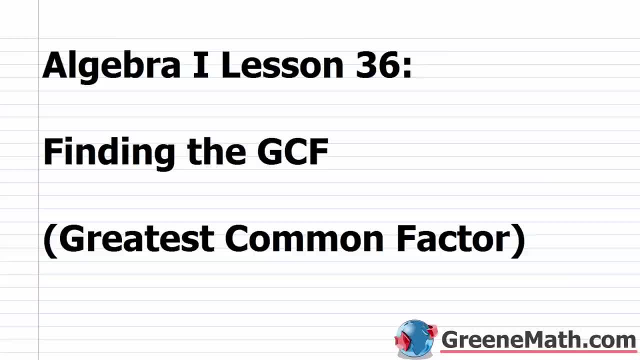 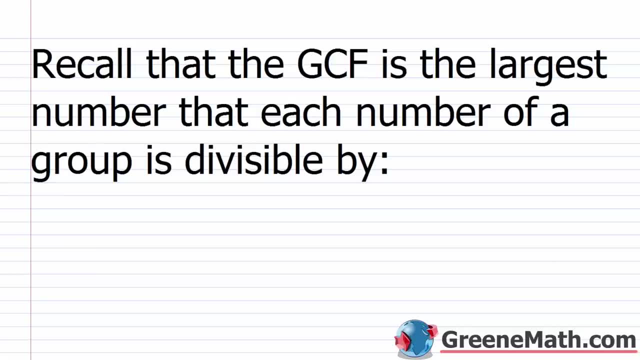 Algebra 1, Lesson 36.. In this video, we're going to learn about finding the GCF, otherwise known as the greatest common factor. So hopefully you learned how to find the greatest common factor in pre-algebra. If this is new to you, I'm going to do enough of a. 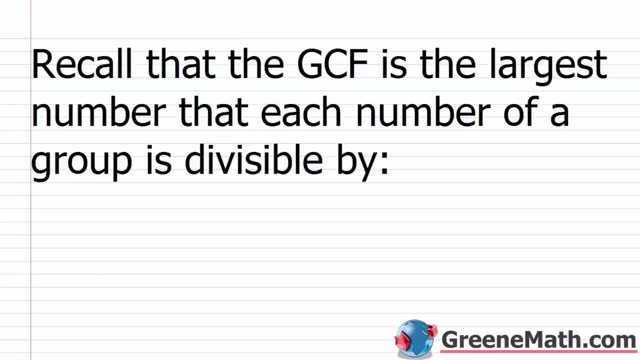 review here, to where you can catch on very quickly. So I want you to recall that the GCF, again, that's the greatest common factor, or some people like to say the greatest common divisor. This is the largest number that each number of a group is. 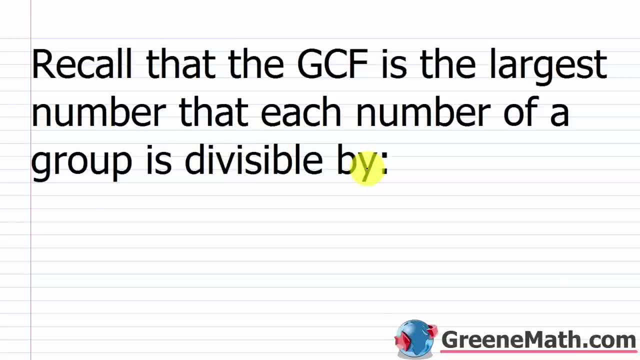 divisible by. So let me give you a quick example. Let's say you had two numbers, let's say 12 and 18.. And I said: what's the largest number? that each number here, 12 and then 18, would be divisible by. Well, what you would do is you would think: 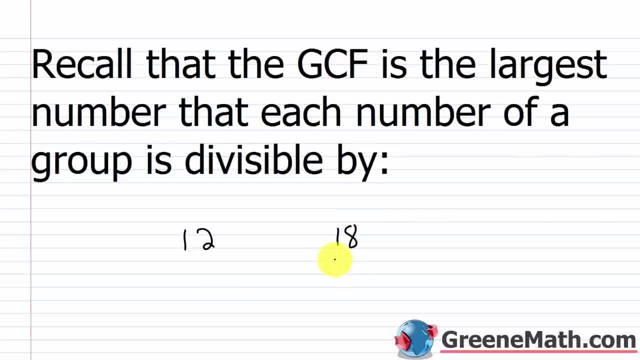 about the factors of each number and then you would find the largest one that's common to both. So for 12, if you think about the factors of 12, you use a factor. here you'd have 4 times 3. 3 is prime, 4 is 2. 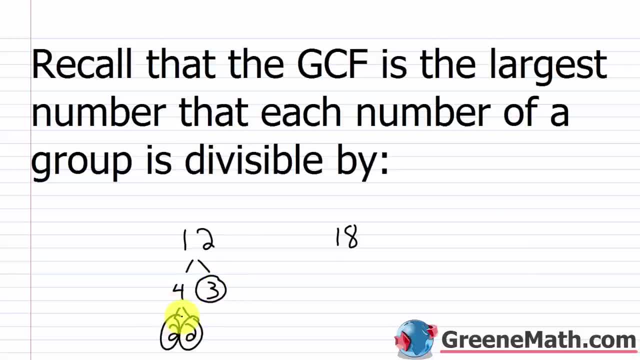 times 2.. So I can think about 12 as 2 times 2 times 3.. So 12 I'm going to think about as 2 times 2 times 3.. And then for 18, if I use a factor tree, I could. 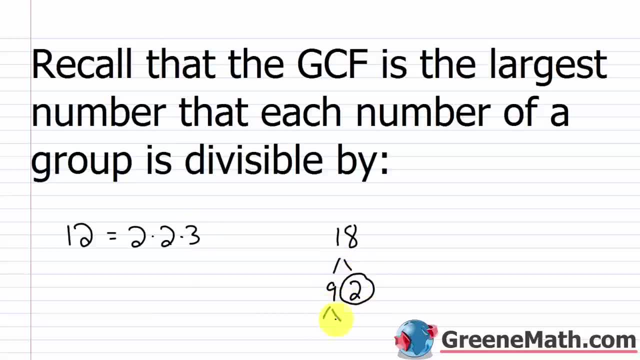 do 9 times 2. 2 is prime, and then 9 is 3 times 3.. 3 is prime. So 18 is 2 times 3 times 3.. So what's common to both? Well, if I look here, I have one factor. 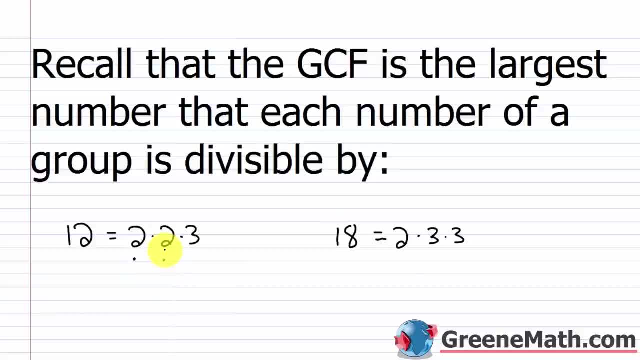 of 2 here and then a second factor of 2 here Over here I only have one factor of 2.. So really, if I was to build a list here, kind of a list, I would think about just putting one factor of 2 in, because that's what's common. 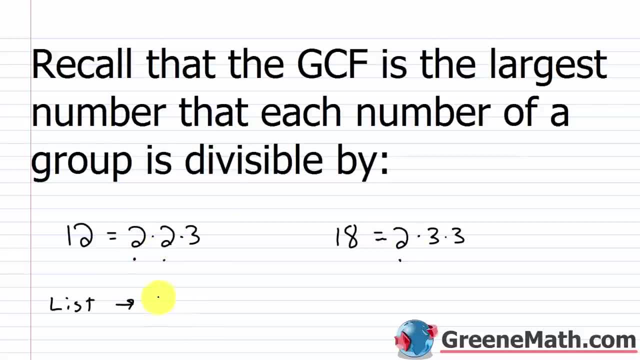 to both. I have 2 here, only 1 here. 1 is common to both, So I'd put a 2 there. Then, if I kind of move on to kind of the next number that's involved, I have a 3 here and then I have. 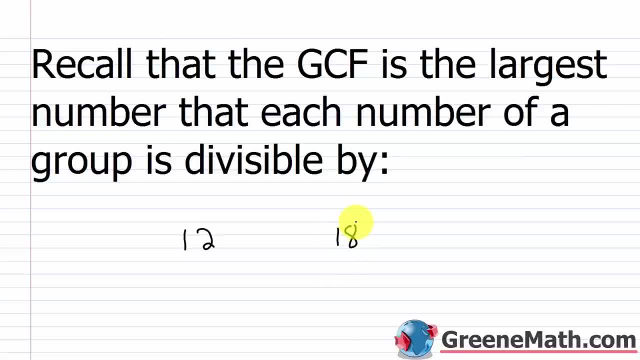 And I said, what's the largest number that each number here, 12 and then 18, would be divisible by? Well, what you would do is you would... You would think about the factors of each number, and then you would find the largest one that's common to both. So for 12, if you think about the factors of 12, you use a factor tree here, you'd have 4x3, 3 is prime, 4 is 2x2. So I can think about 12 as 2x2x3. So 12, I'm going to think about as 2x2x3. And then for 18, if I use a factor tree, I could do 9x2x3. 2 is prime, and then 9 is 3x3. 3 is prime. So 18 is 2x3x3. 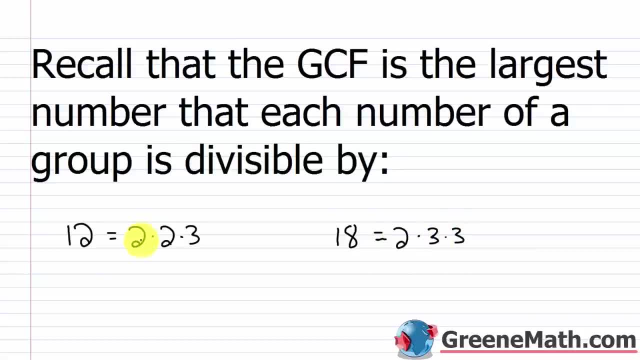 So what's common to both? Well, if I look here, I have one factor of 2 here, and then a second factor of 2 here. Over here, I only have one factor of 2. 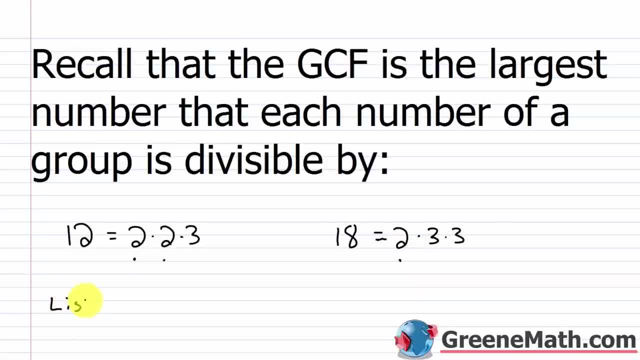 So really, if I was to build a list here, kind of a list, I would think about just putting one factor of 2 in. What's common to both? I have 2 here, only 1 here, 1 is common to both. So I'd put a 2 there. 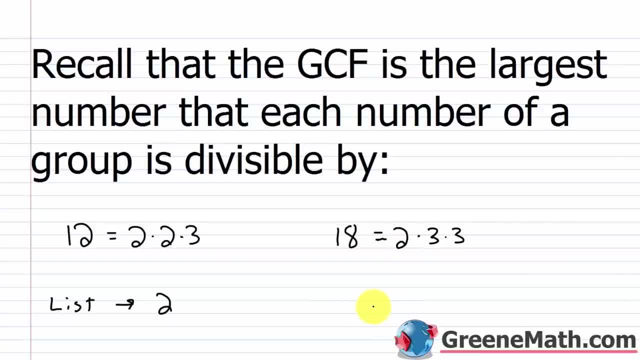 Then, if I kind of move on to kind of the next number that's involved, I have a 3 here, and then I have 1, 3, 2 3s here. 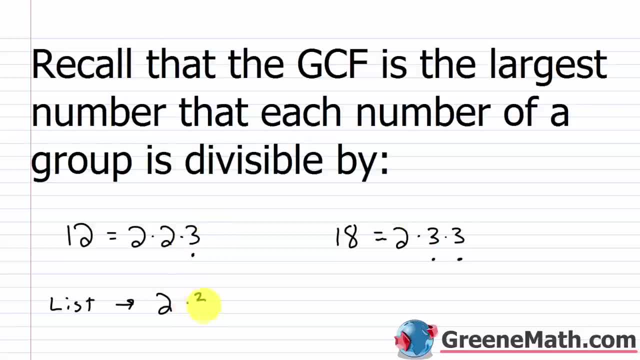 So 1, 3 is common to both. So times 3. So my list would contain 1, 2, and 1, 3. 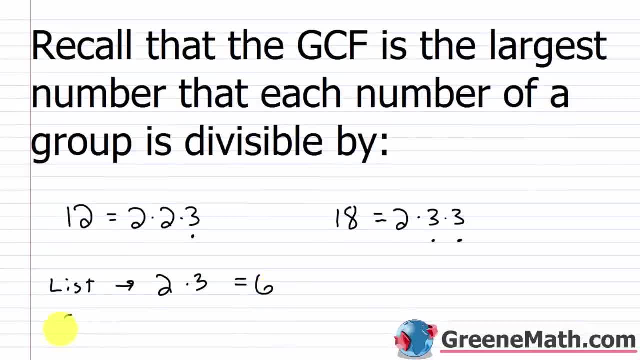 I'd multiply them together to get 6. And so the GCF is the number 6. Right? And you can see if you took 12 and you divide it by 6, you get 2. Right? 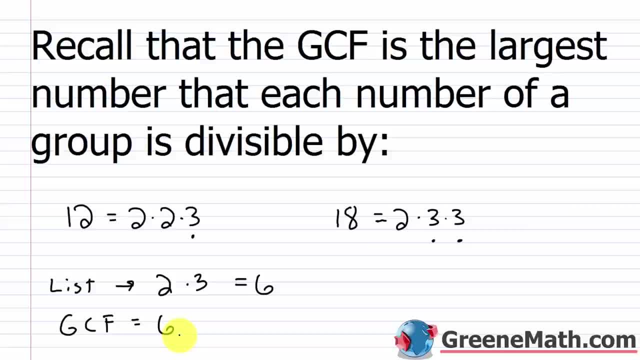 Remember, if we talk about something being divisible by something, then that means it divides evenly. There's no remainder. So 12 divided by 6 is 2. No remainder. 18 divided by 6 is 3. No remainder. 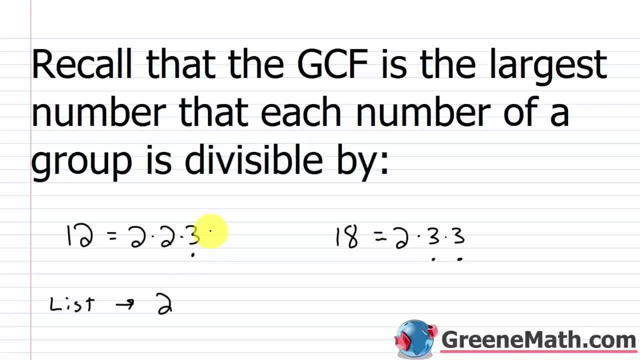 1, 3, 2, 3's here, So 1, 3 is common to both, So times 3, So my list would contain 1, 2 and 1, 3.. I'd multiply them together to get 6.. 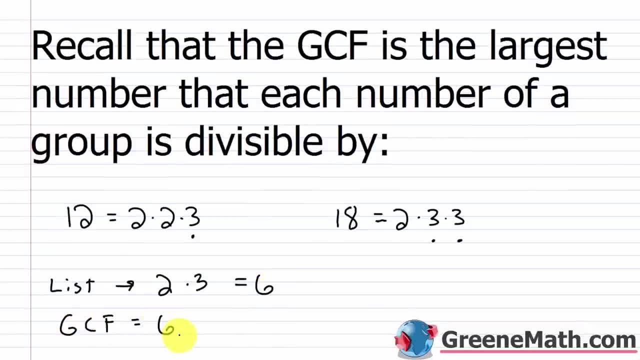 And so the GCF is the number 6.. And you can see: if you took 12 and you divide it by 6, you get 2.. Remember, if we talk about something being divisible by something, then that means it divides evenly. there's no remainder. So 12 divided by 6. 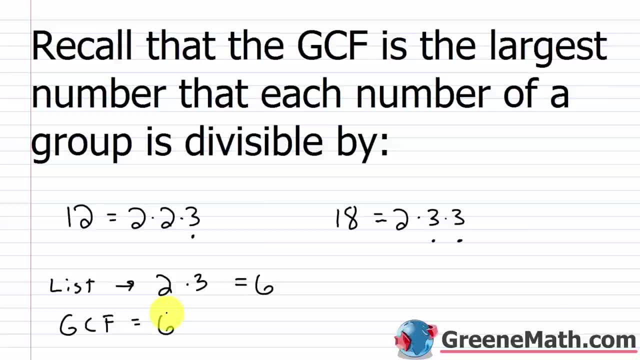 is 2, no remainder. 18 divided by 6 is 3, no remainder. So that is the largest number that each number of this group, the 12 and the 18, would be divisible by. So let's go over the official. 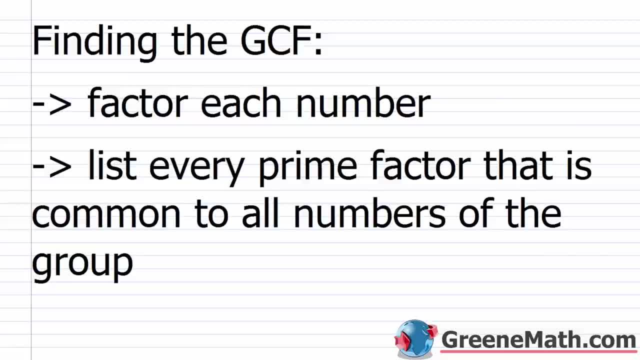 procedure for finding the GCF And once you kind of get good at this, you don't need to do all the work that I just did, or even the work that you do in this kind of procedure. In most cases, if the numbers that you're working with 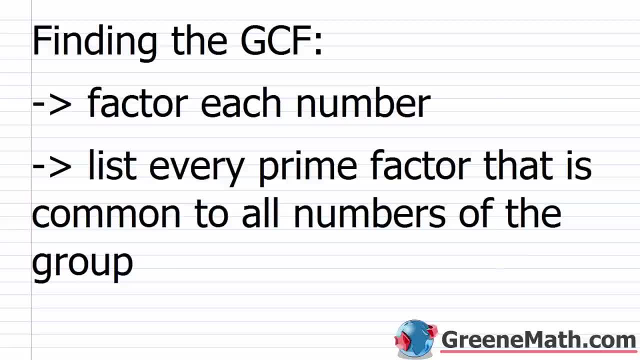 are small enough you can pretty much eyeball it and see what the GCF is going to be. So I want you to factor each number completely. So you can do that with a factor tree or you can do it using kind of any method that you've learned. 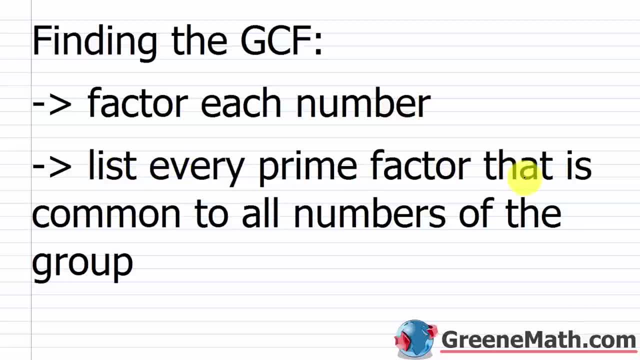 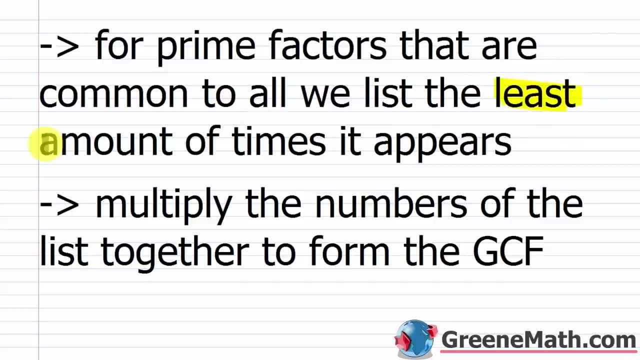 Then you want to list every prime factor that is common to all numbers, All numbers of the group. Okay, So it's got to be common to everything. Then, for prime factors that are common to all, we list the least, the least amount of times. 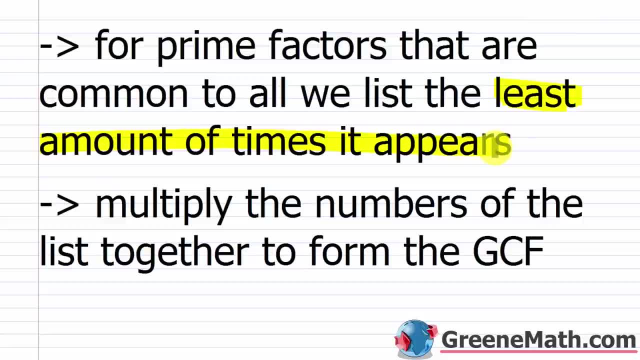 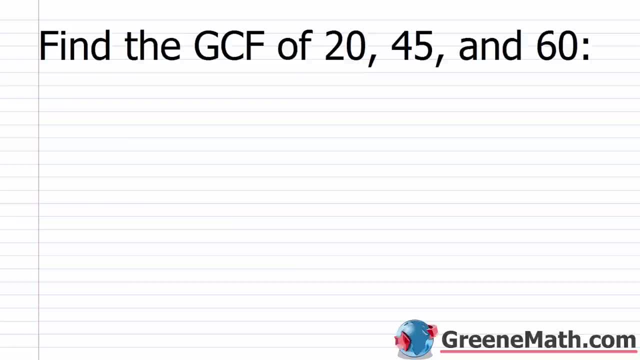 it appears. So once you've done this, you're just going to multiply the numbers of the list together to form the GCF. Alright, so let's take a look at an example here. So we want to find the GCF of 20,. 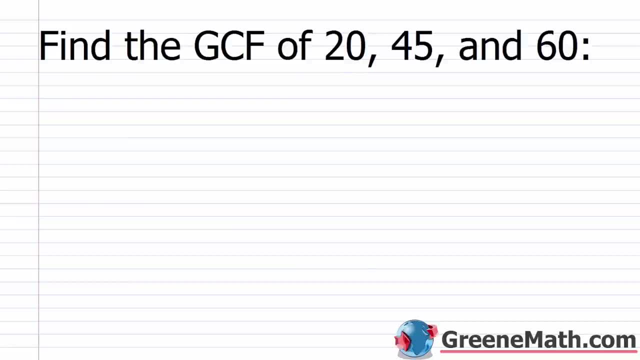 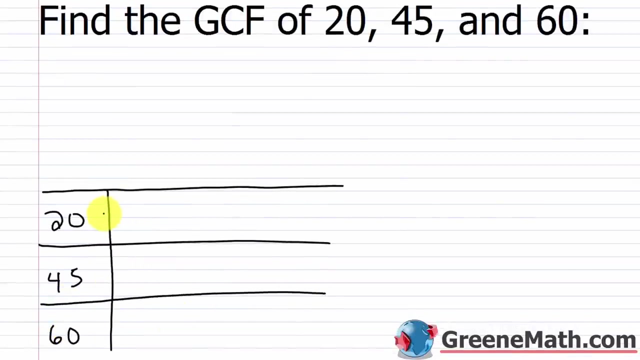 45, and 60. So kind of the best way I've found for students to kind of completely understand this, I just build a little table. So my table will consist of the prime factors for 20 and 45 and 60. So I'm going to put equals. 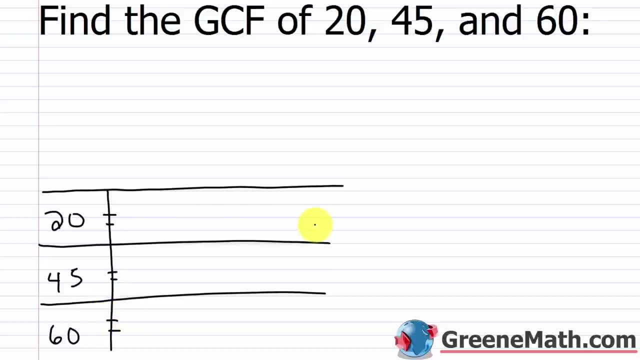 and then I'll list my prime factors here. So to do that I'm just going to use a factor tree in each case. So for 20, I can start out by saying 4 times 5. I know 5 is prime, so I'm going to circle that. 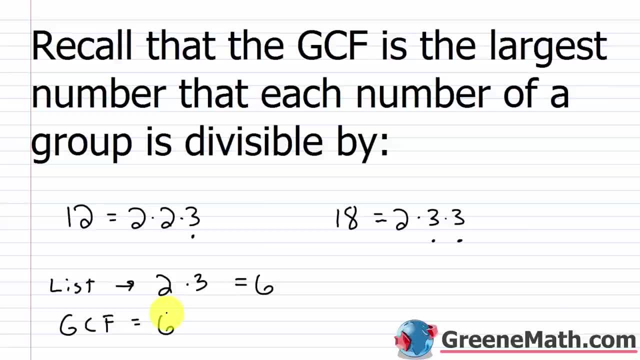 So that is the largest number that each number of this group, the 12 and the 18, would be divisible by. All right. 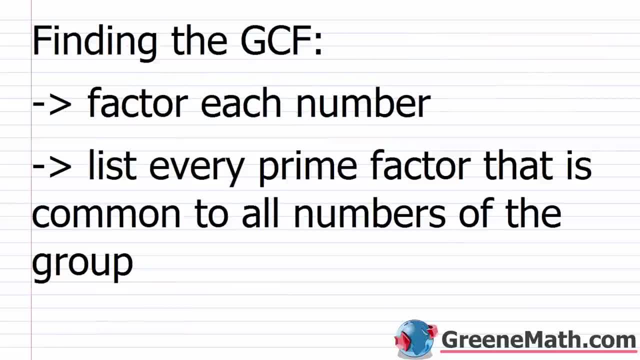 So let's go over the official procedure for finding the GCF. 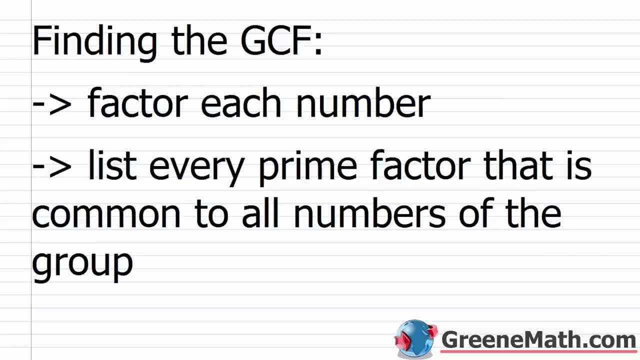 And once you kind of get good at this, you don't need to do all the work that I just did, or even the work that you do in this kind of procedure. 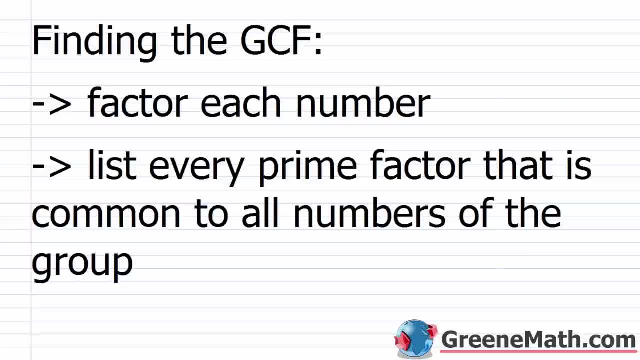 In most cases, if the numbers that you're working with are small enough, you can pretty much eyeball it and see what the GCF is going to be. 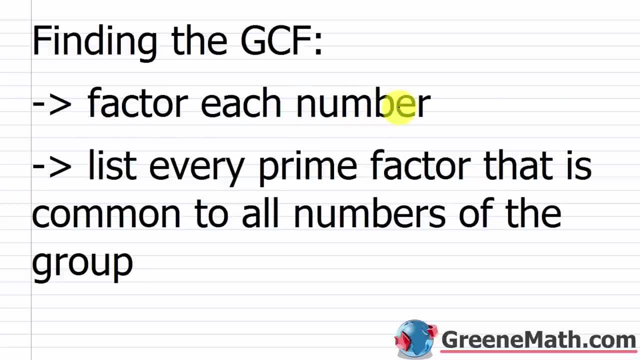 So I want you to factor each number completely. So you can do that with a factor tree, or you can do it using kind of any method that you've learned. 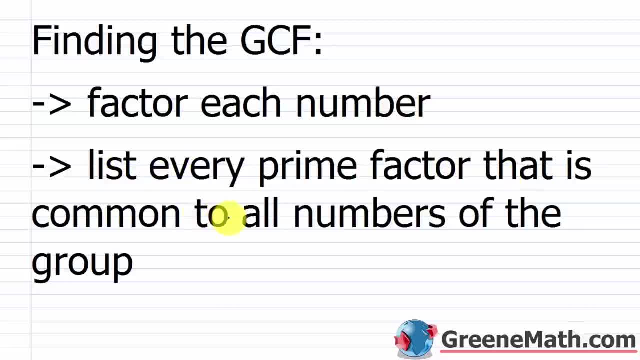 Then you want to list every prime factor that is common to all numbers. All numbers of the group. Okay. So it's got to be common to everyone. Everything. 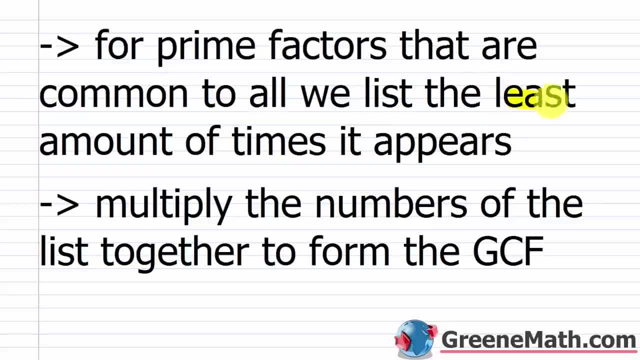 Then for prime factors that are common to all, we list the least, the least amount of times it appears. So once you've done this, you're just going to multiply the numbers of the list together to form the GCF. All right. So let's take a look at an example here. 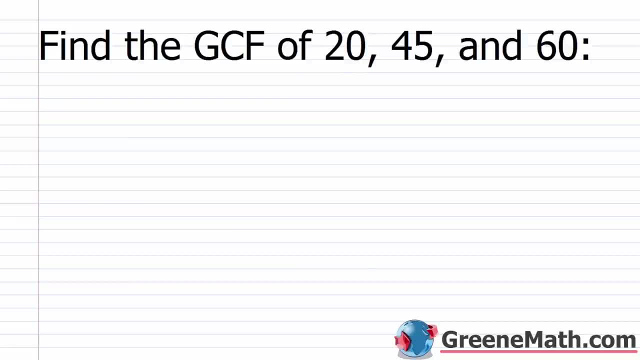 So we want to find the GCF of 20, 45, and 60. So kind of the best way I've found for students to kind of completely understand this, I just build a little table. 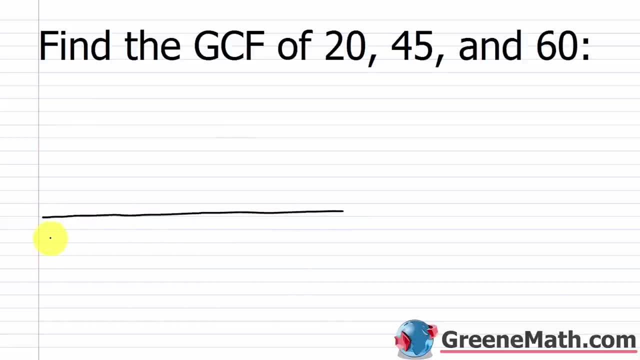 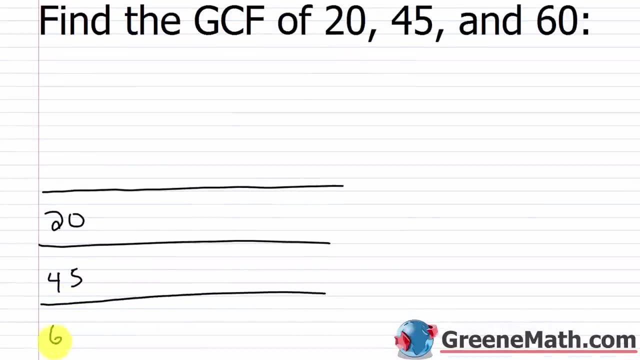 So my table will consist of the prime factors for 20, and 45, and 60. So I'm going to put equals, and then I'll list my prime factors here. 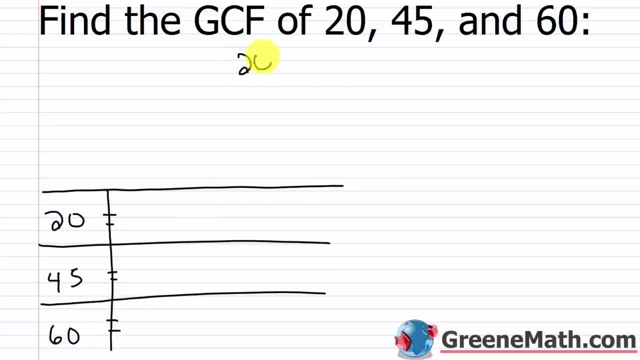 So to do that, I'm just going to use a factor tree in each case. So for 20, I can start out by saying 4 times 5. I know 5 is prime, so I'm going to circle that. And then 4, I know I can write as 2 times 2. 2 is prime, so I'll go ahead and circle both of those. So then the next one I have is 45. So 45, and I can start out by saying 9 times 5. And again, 5 is prime, so let's circle that. And then for 9, I would split that up into 3 times 3. 3 is prime. Let's go ahead and circle both of those. 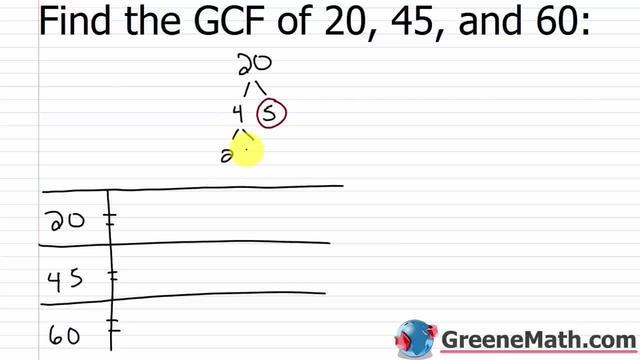 And then 4. I know I can write as 2 times 2.. 2 is prime, so I'll go ahead and circle both of those. So then the next one I have is 45.. So 45, and I can start out by saying: 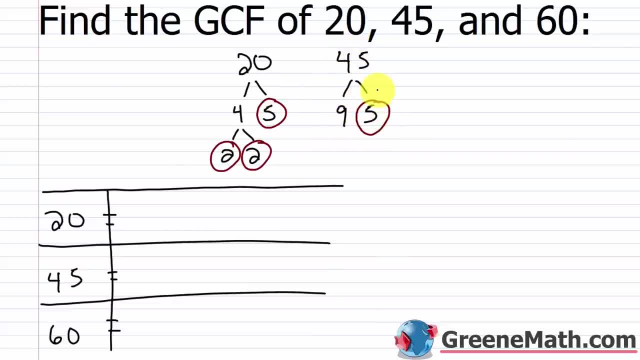 9 times 5.. And again, 5 is prime. so let's circle that, And then for 9, I would split that up into 3 times 3.. 3 is prime. let's go ahead and circle both of those And then the last. 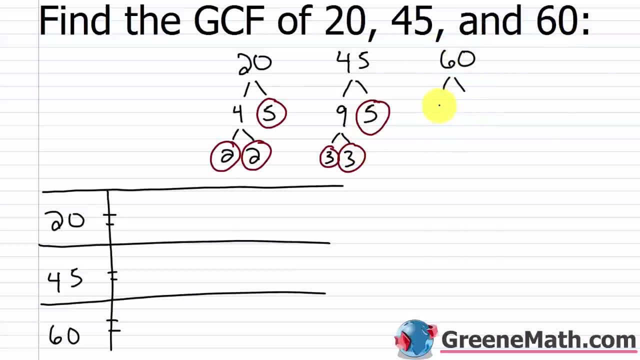 one is 60. So for 60 I can do 6 times 10.. 6 is 2 times 3. And 2 and 3 are both prime, so let's circle those, And then for 10 we do 5. 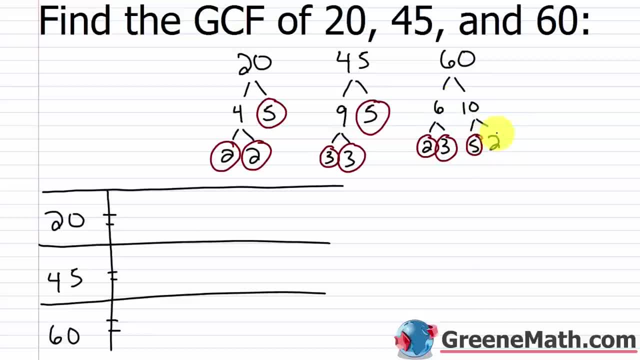 times 2.. And 5 and 2 are both prime, so we'll circle those Alright. so I'm going to write this in this table in such a way to where it's completely obvious what's common to everything. So for 20, the smallest prime, 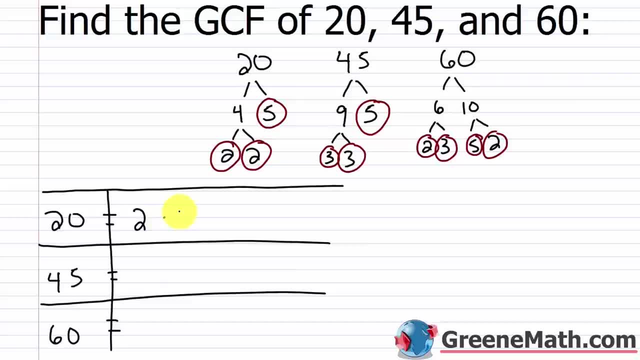 factor is 2, so let's go ahead and start out with that. So we have 2 times 2 and then I have times 5, but I'm going to put that way out here. I'll put that way out here For 45. I. 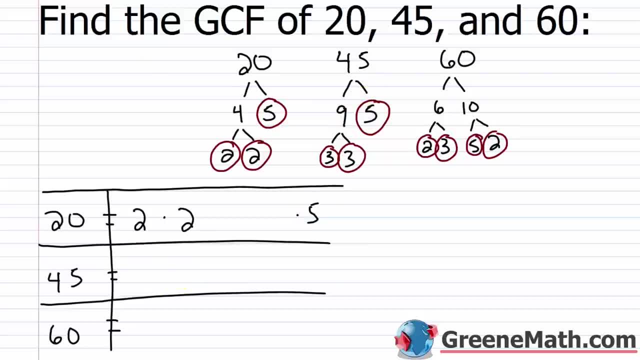 don't have any factors of 2.. So I'm going to kind of mark those out to show that it's not here, not here. And then I have 1,, 2 factors of 3. So let's put that there. So times 3. 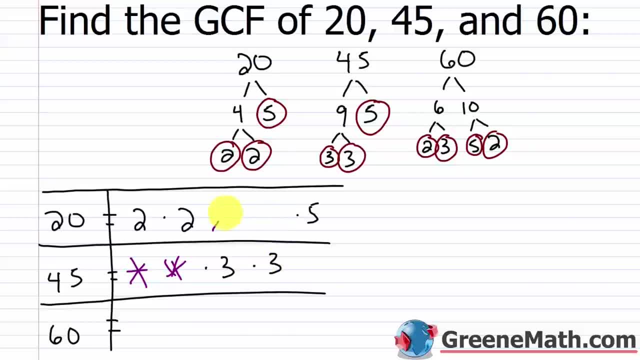 times 3.. And while I'm doing this, I'm going to go ahead and mark this out to show I don't have that here. It's not going to be common to everything. And then I also have a factor of 5 in 45, so times 5.. 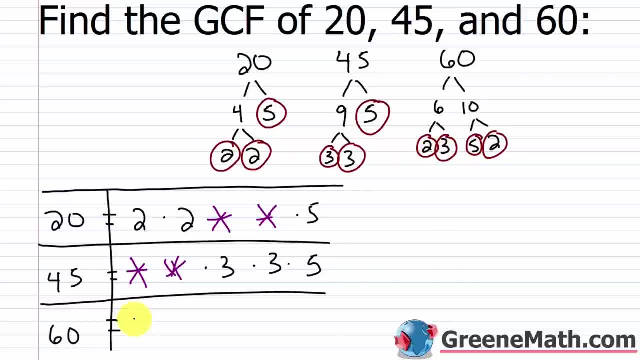 Now for 60. I have 2 factors of 2.. 2 times 2.. I have 1 factor of 3, but I don't have a second factor of 3, so I'm going to mark that out. And then I have 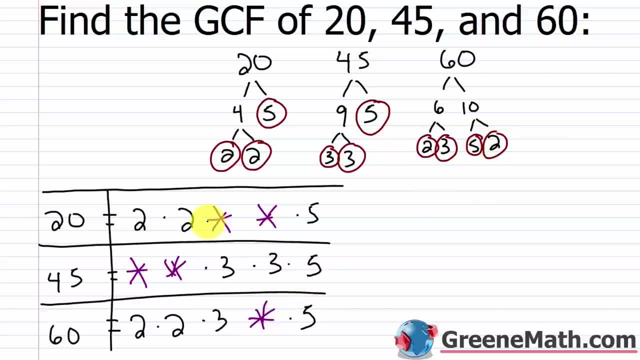 1 factor of 5.. 1 factor of 5.. So when we kind of look at this table here, it makes it completely obvious what's going to be common to everything. So, starting out with kind of 20, I have 2 factors of 2, but I don't have 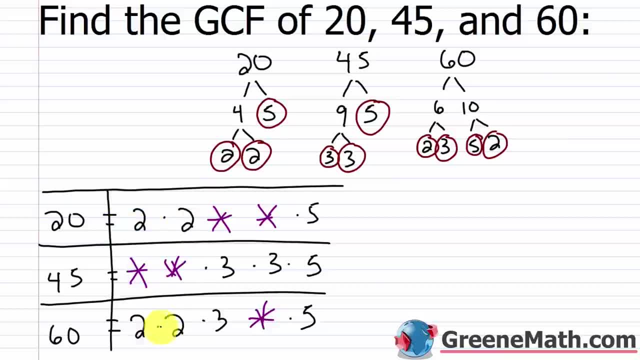 any factors of 2 in 45, even though I have 2 factors of 2 in 60,. 2 wouldn't go in the list when I go to build my GCS Because it's not common to everything Moving on. I don't have any factors of. 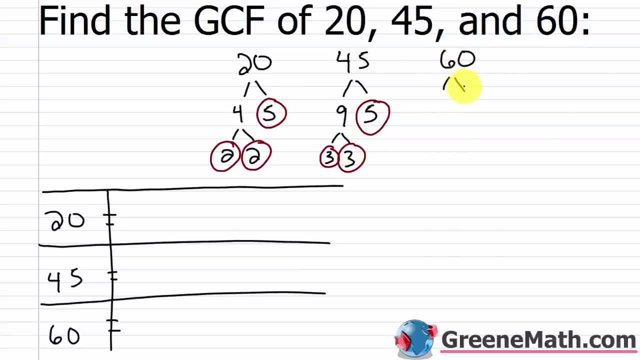 And then the last one is 60. So for 60, I can do 6 times 10. 6 is... 6 is 2 times 3. And 2 and 3 are both prime, so let's circle those. 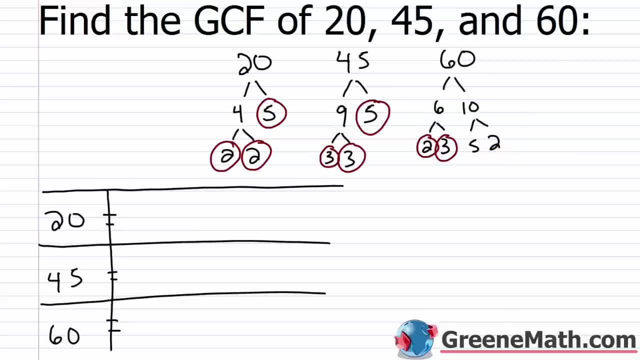 And then for 10, we do 5 times 2. And 5 and 2 are both prime, so we'll circle those. 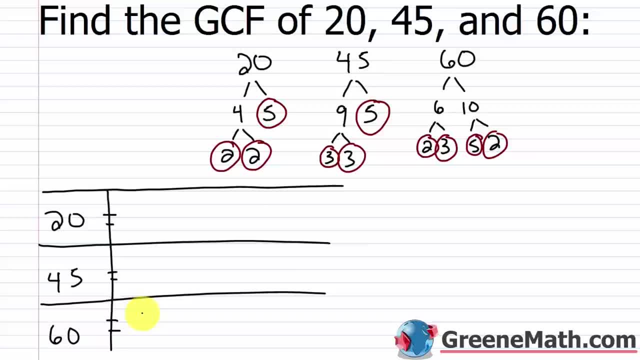 All right, so I'm going to write this in this table in such a way to where it's completely obvious what's common to everything. So for 20, the smallest prime factor is 2. So let's go ahead and start out with that. 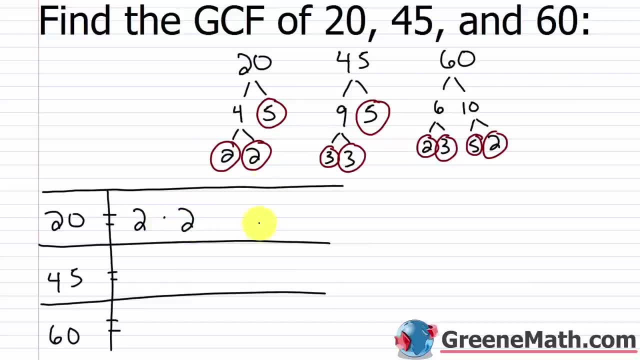 So we have 2 times 2. And then I have times 5, but I'm going to put that way out here. I'll put that way out here. For 45, I don't have to do that. I don't have any factors of 2. 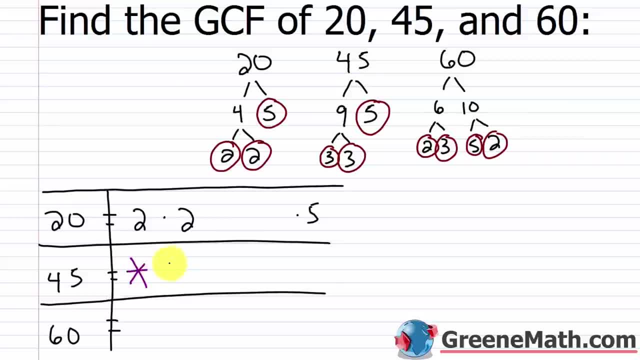 So I'm going to kind of mark those out to show that it's not here, not here. And then I have 1, 2 factors of 3. So let's put that there. 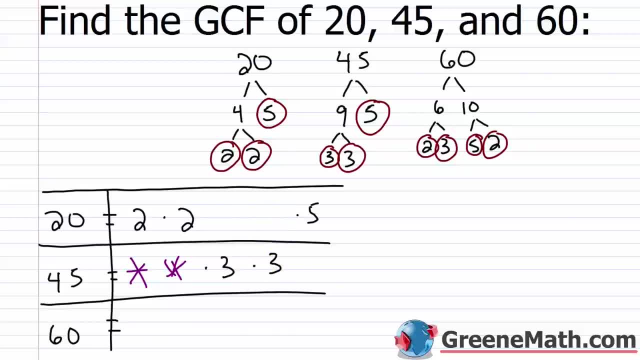 So times 3, times 3. And while I'm doing this, I'm going to go ahead and mark this out to show I don't have that here. It's not going to be common to everything. 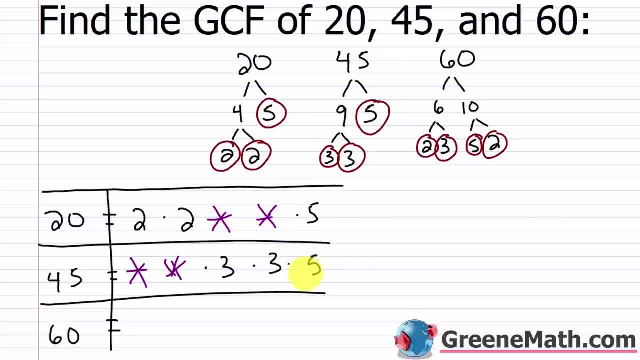 And then I also have a factor of 5 in 45, so times 5. Now for 60, I have 2 factors of 2. So 2 times 2. 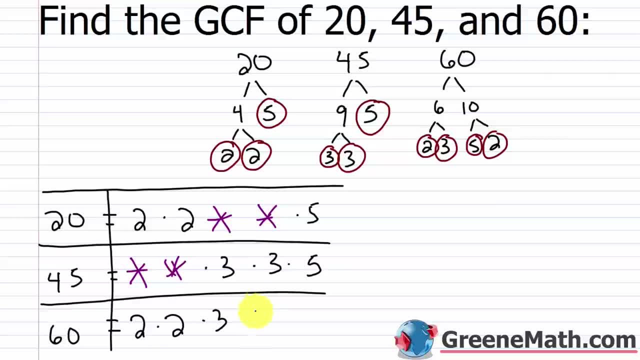 I have 1 factor of 3, but I don't have a second factor of 3. So I'm going to mark that out. 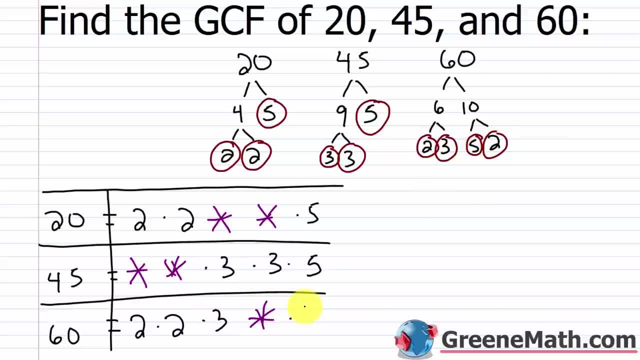 And then I have 1 factor of 5. 1 factor of 5. 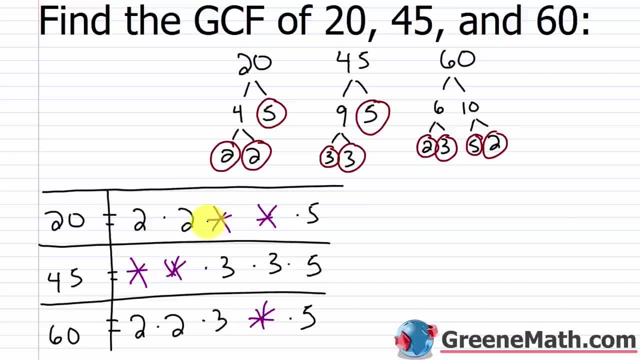 So when we kind of look at this table here, it makes it completely obvious what's going to be common to everything. 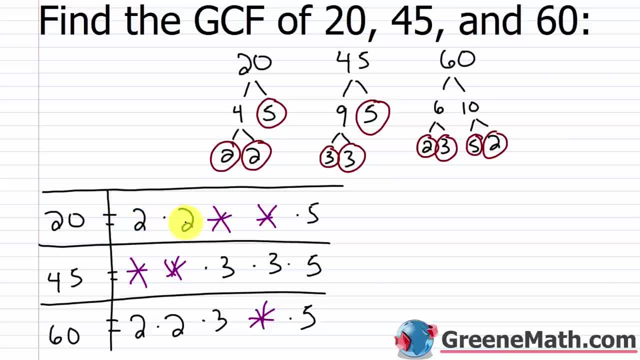 So starting out with kind of 20, I have 2 factors of 2. But I don't have any factors of 2 in 45. 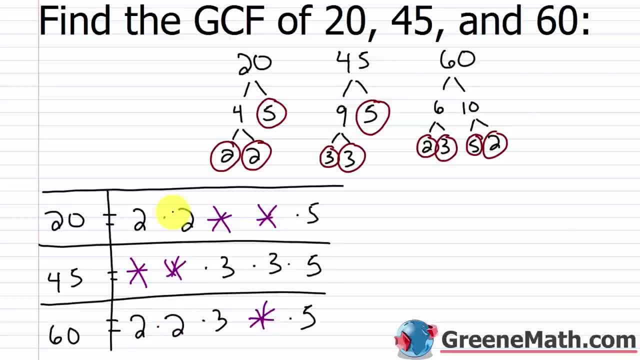 Even though I have 2 factors of 2 in 60, 2 wouldn't go in the list when I go to build my GCF. 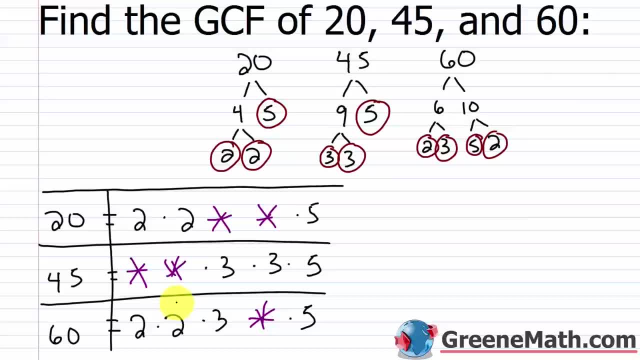 Because it's not common. It's common to everything. Okay? 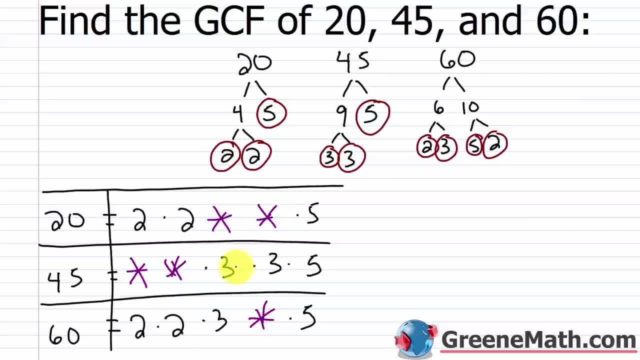 Moving on, I don't have any factors of 3 up here. Even though I have 2 factors of 3 here, and 1 factor of 3 here. 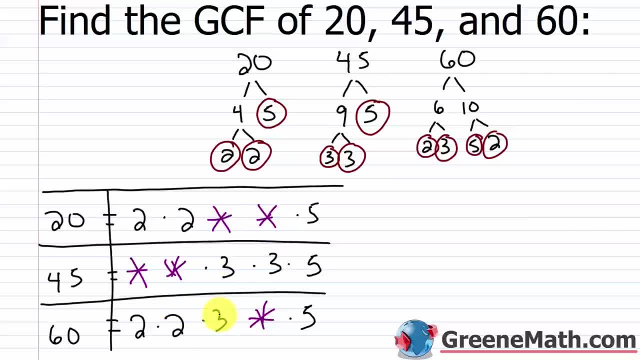 3 up here, even though I have 2 factors of 3 here and 1 factor of 3 here. Because there's no factors of 3 in the prime factorization of 20, it doesn't go in the list either. It's got to be common to. 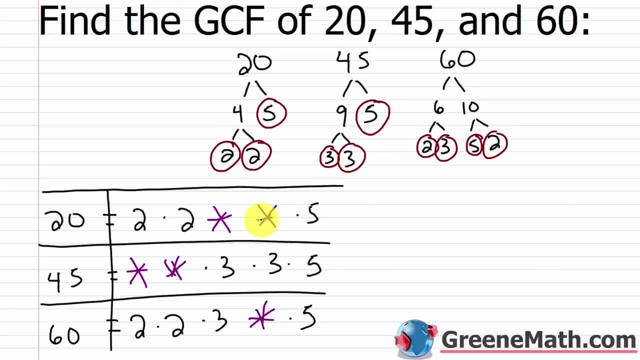 everything. The only number that's common to every prime factorization is 5.. So I want to highlight that There's a 5 in each prime factorization and there's only one of those, So my GCF here would just be the number 5.. 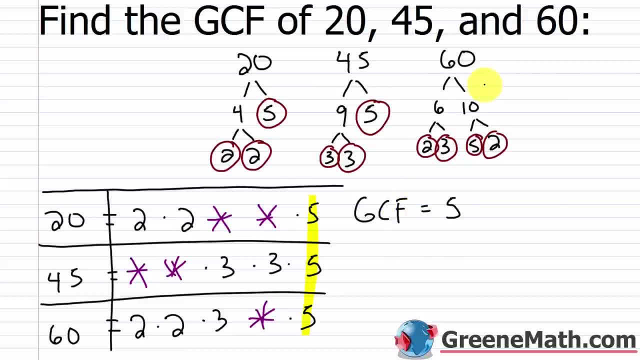 And go ahead and take each number here and divide it by 5.. You'll see that you don't get a remainder and you won't be able to find any number that's larger than 5. that each number of the group is divisible by 5 is 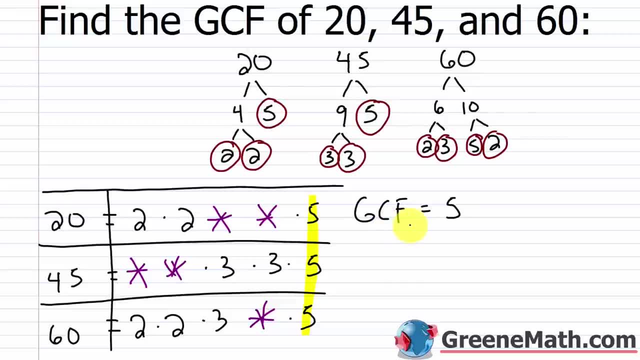 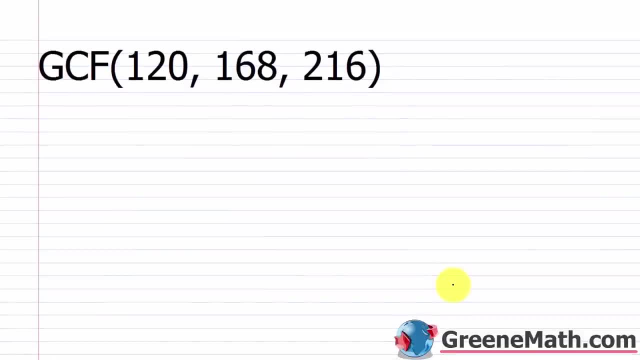 the largest one, and so that's our greatest common factor, or a lot of you will hear this called the greatest common divisor. Alright, let's take a look at it all. So we want to find the greatest common factor of 120, 168 and 216.. 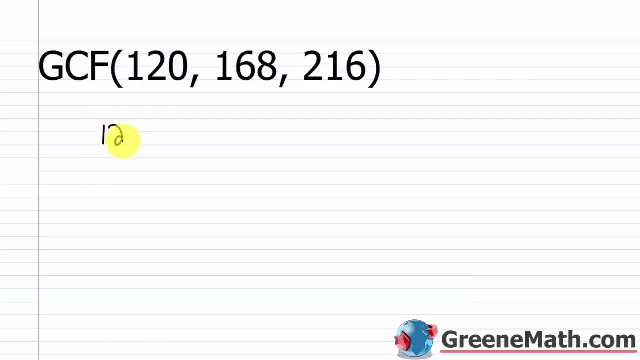 So again, I'm just going to factor each one, So 120, and I'm going to start out, because it says a 0 at the end. I know it's divisible by 10, so I'm just going to go 12 times 10.. 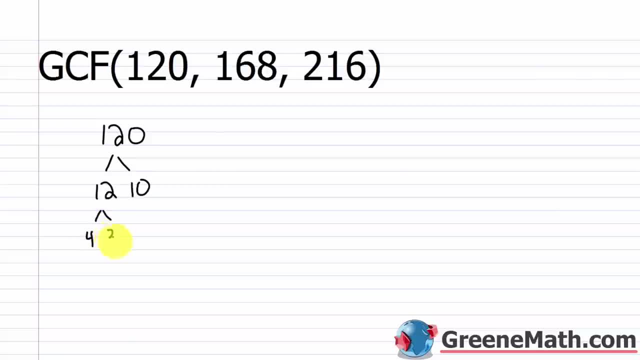 I'm going to start out with that 12 I can do 4 times 3, and 3 is prime, 4 is going to be 2 times 2 and 2 is prime For 10. I'm going to write that as 5 times 2.. 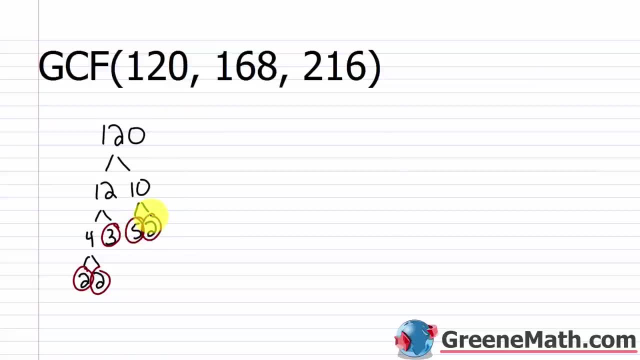 5 and 2 are both prime. Alright, so that one's done. So let's do 168 now. So what are two factors of 168? to kind of get started, It's an even number, so I know it's divisible by 2. 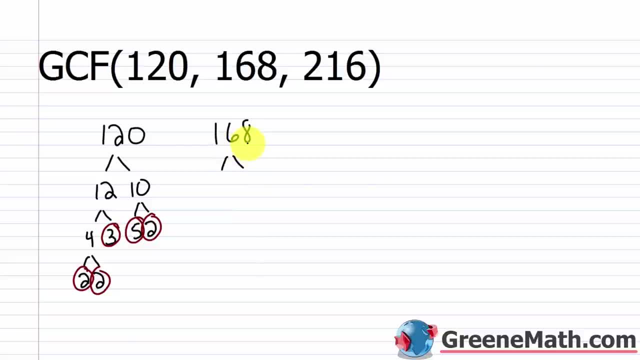 but also I know that the final two digits here, 68, would be divisible by 4. so therefore the number is So: what is 168 divided by 4?? Well, that's going to be 42. So I know this would be 42. 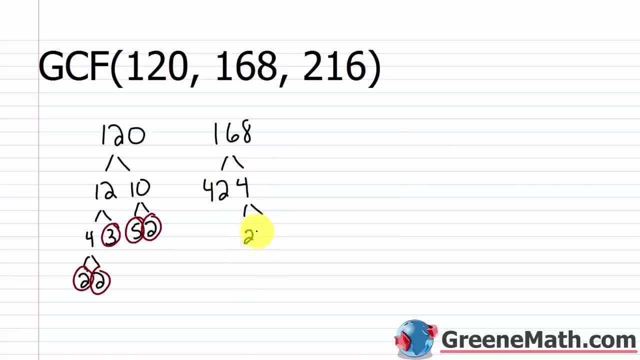 times 4 to start, and 4 is easy. that's 2 times 2.. Both of those are prime. We'll circle them For 42. we know we can do 7 times 6. That's easy. from watching football, Your team scores. 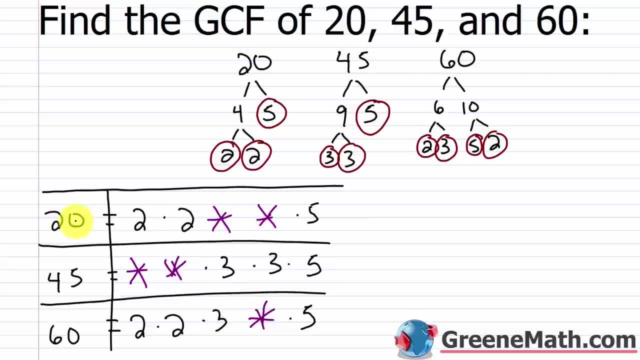 Because there's no factors of 3 in the prime factorization of 20, it doesn't go on the list either. 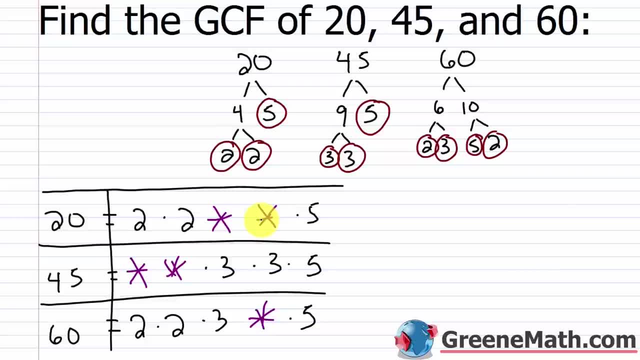 It's got to be common to everything. The only number that's common to every prime factorization is 5. 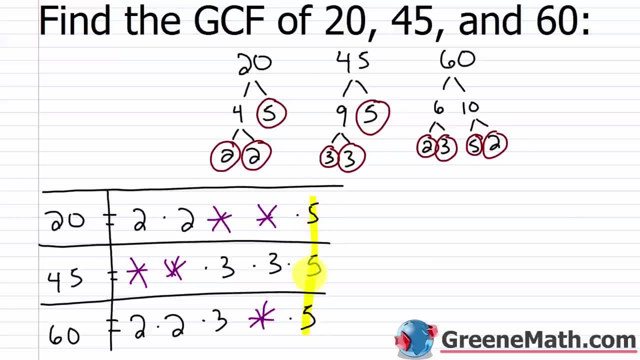 So I want to highlight that. There's a 5 in each prime factorization. And there's only one of those. So my GCF here, would just be the number 5. 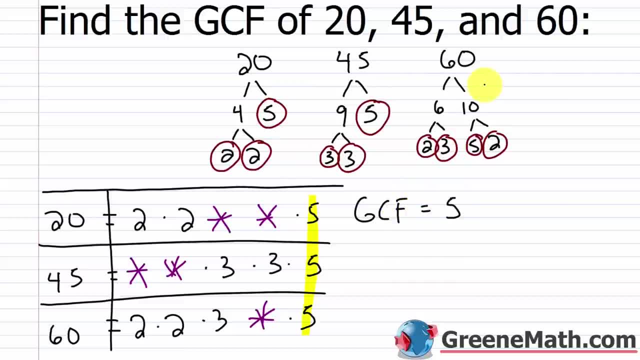 And go ahead and take each number here and divide it by 5. You'll see that you don't get a remainder. 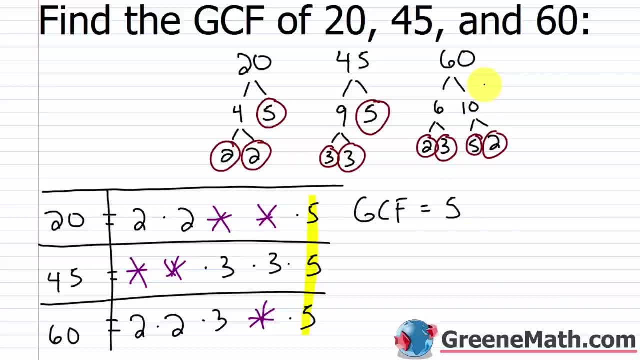 And you won't be able to find any number that's larger than 5, that each number of the group is divisible by. 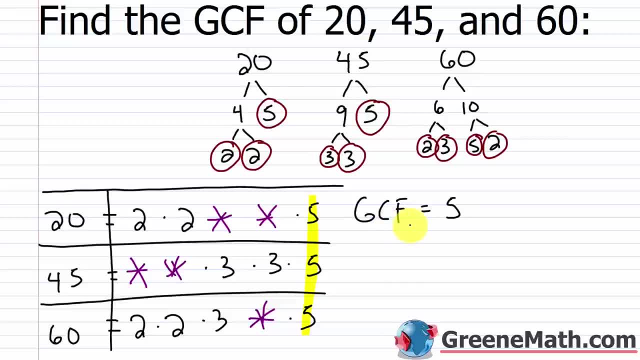 Alright, 5 is the largest one. And so that's our greatest common factor, or a lot of you will hear this called the greatest common divisor. 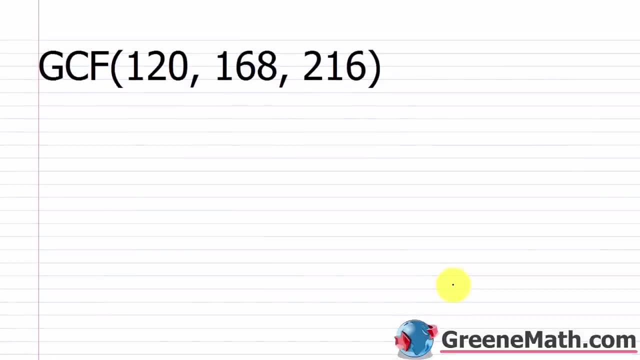 Alright, let's take a look at it all. So we want to find the greatest common factor of 120, 168, and 216. So again, I'm just going to factor each one. 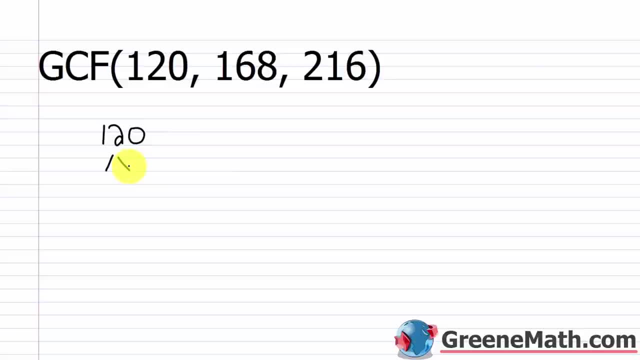 So 120. And I'm going to start out, because it says a 0 at the end, I know it's divisible by 10. So I'm just going to go 12 times 10. I'm going to start out with that. 12, I can do 4 times 3. And 3 is prime. 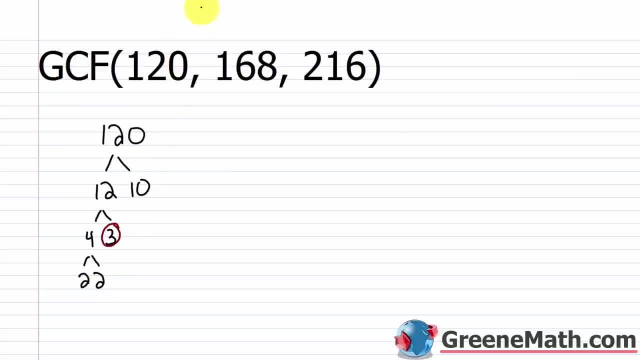 4 is going to be 2 times 2. And 2 is prime. For 10, I'm going to write that as 5 times 2. 5 and 2 are both prime. Alright, so that one's done. So let's do 168 now. 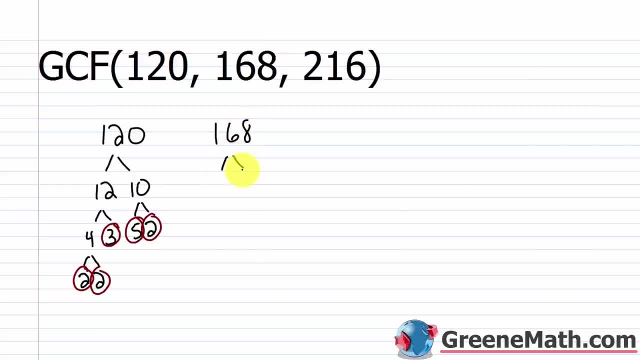 So what are two factors of 168 to kind of get started? It's an even number, so I know it's divisible by 2. But also, I know that the final two digits here, 68, would be divisible by 4. So therefore, the number is. 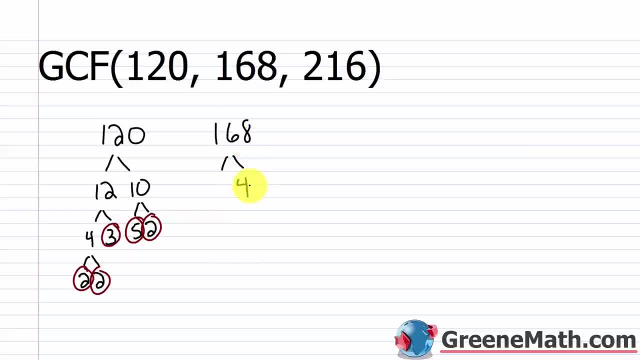 So what is 168 divided by 4? Well, that's going to be 42. 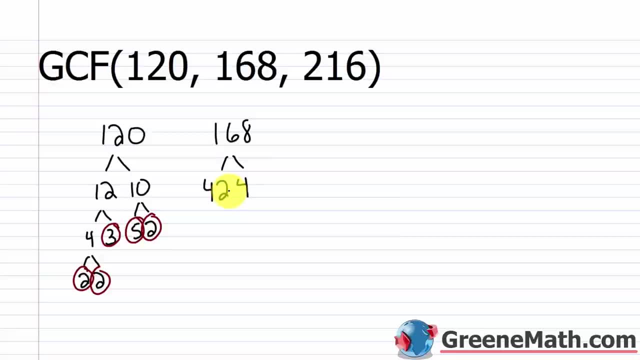 So I know this would be 42 times 4 to start. And 4 is easy. That's 2 times 2. Both of those are prime. We'll circle them. 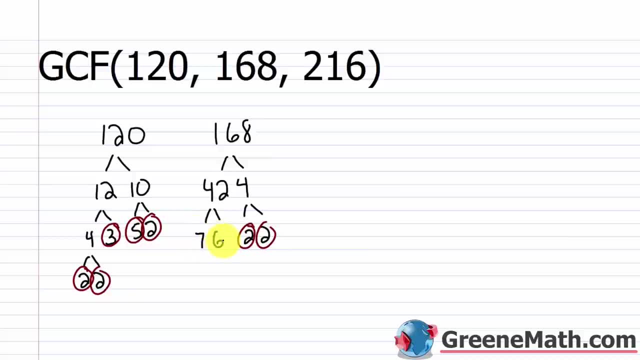 For 42, we know we can do 7 times 6. That's easy from watching football. 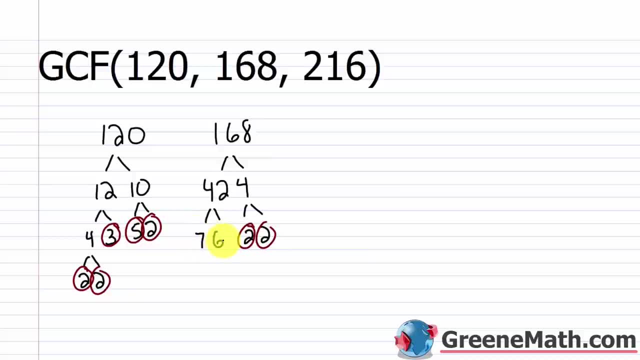 Your team scores 6 touchdowns with 6 extra points. They have 42 points. 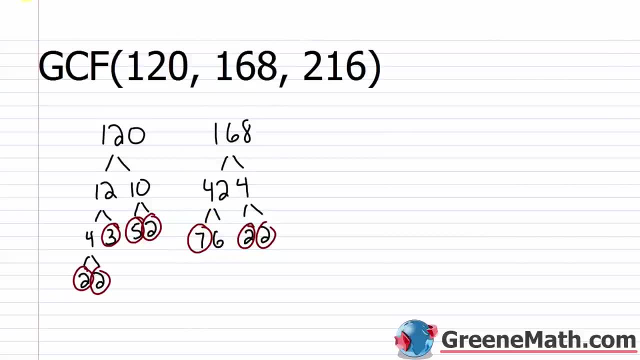 So then 7 is a prime number. We'll circle that. And then for 6, that is 3 times 2. And both those are prime. So we'll circle those. OK. So now we want 216. 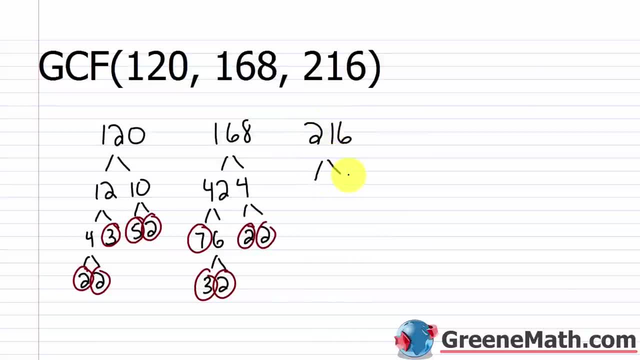 Again, it's an even number. And also, 60. 16 is divisible by 4. So that means 216 would be. 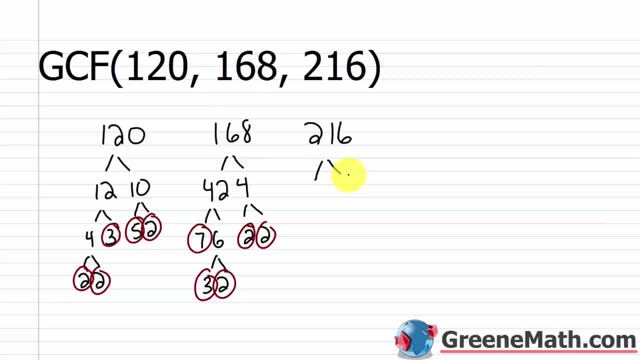 So let's go ahead and start out with 54 times 4. 54 times 4. 4, again, is 2 times 2. And 2 is prime. So we'll circle those. 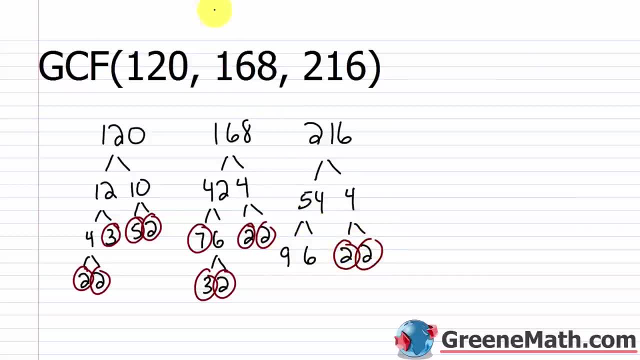 And for 54, I know that's 9 times 6. And 9, 3 times 3. 3 is prime. Let's circle those. 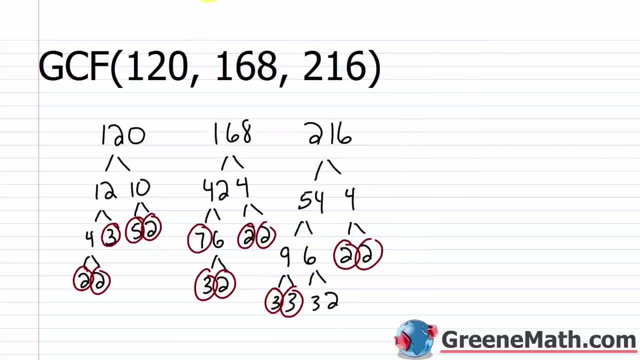 And for 6, 3 times 6. Or 6, 3 times 2. Again, 3 and 2 are both prime. So let's circle those. OK. 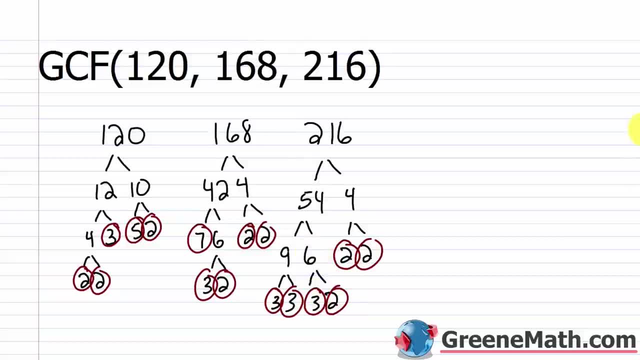 So now that we've got this set up, let's go ahead and make a table. Let's go ahead and make a table just like we did in the last example. So we're going to make four lines here. 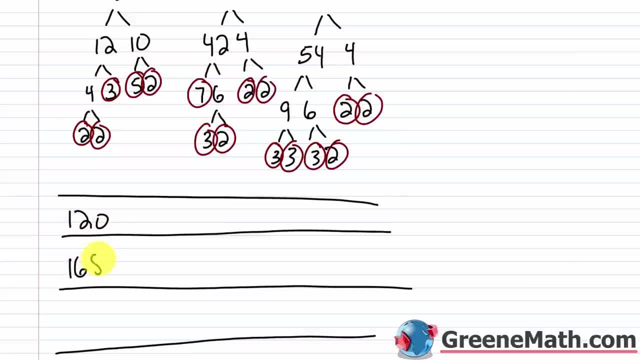 OK. So we'll have 120, 168, and 216. Put a little line there. OK. 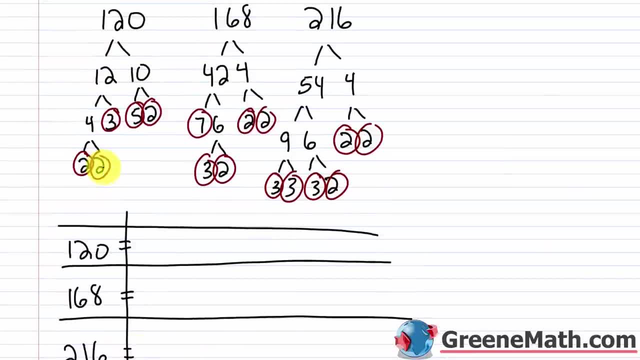 So the prime factorization for 120. I have 2 times 2 times 2. 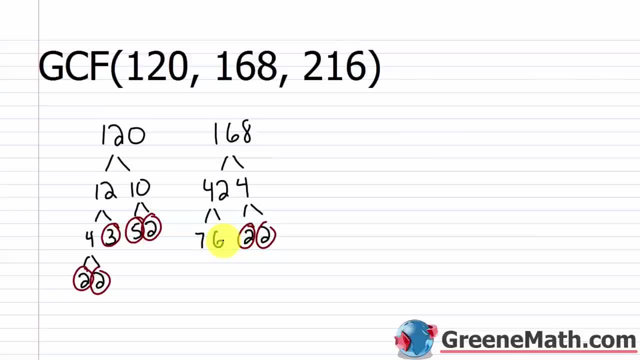 6 touchdowns with 6 extra points, They have 42 points. So then 7 is a prime number. We'll circle that. and then for 6, that is 3 times 2, and both those are prime, so we'll circle those. 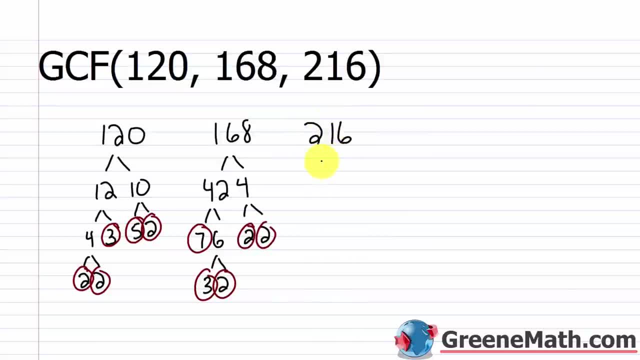 So now we want 216.. Again, it's an even number, and also 16 is divisible by 4, so that means 216 would be. So let's go ahead and start out with 54 times 4.. 54 times 4.. 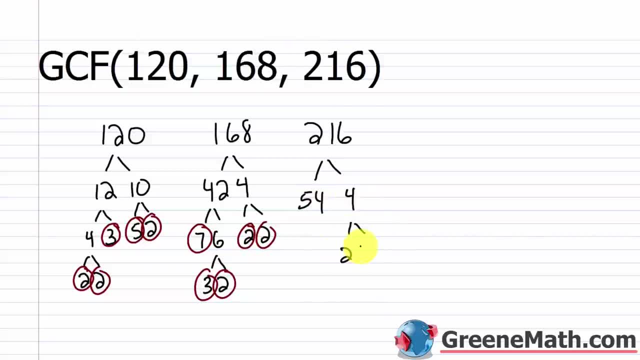 4 again is 2 times 2.. And 2 is prime, so we'll circle those. And for 54, I know that's 9 times 6 and 9, 3 times 3.. 3 is prime. Let's circle those. 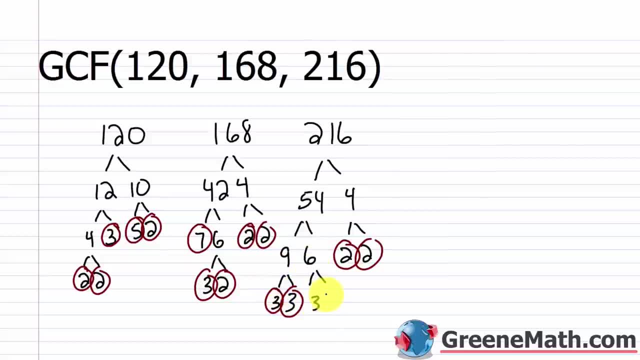 And for 6, 3 times 2.. Again, 3 and 2 are both primes, So let's circle those, Okay? so now that we've got this set up, let's go ahead and make a table. Let's go ahead and make a table, just like we did. 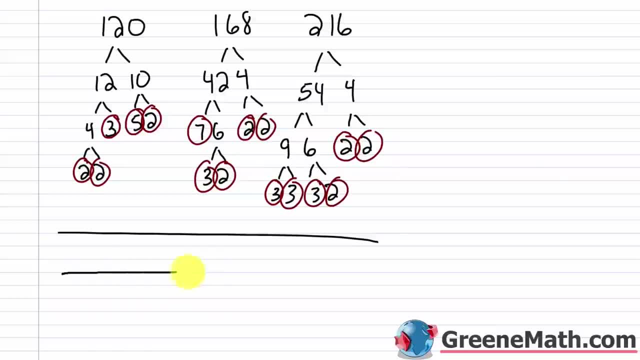 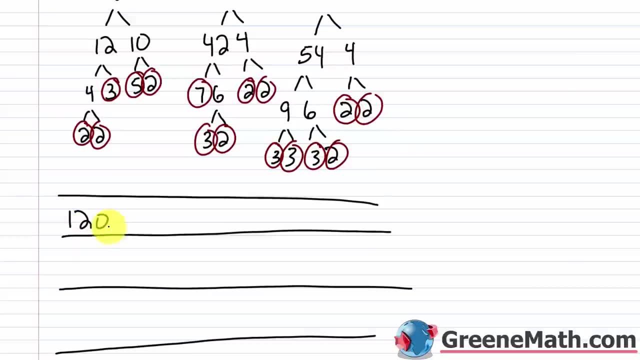 in the last example. So we're going to make 4 lines here. Okay, so we'll have 120,, 168, and 216.. Put a little line there, Okay so prime factorization for 120.. I have 2 times, 2 times 2.. 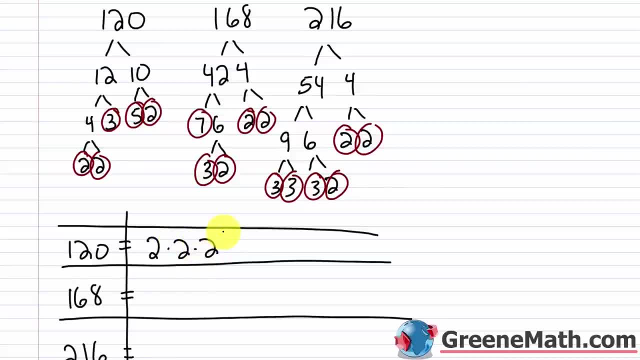 2 times 2 times 2.. And let me kind of look at 168 now. So I have 2 times 2 times 2.. So I have 3 factors of 2 there as well, And then in 216 I have 3 factors of 2 as well. 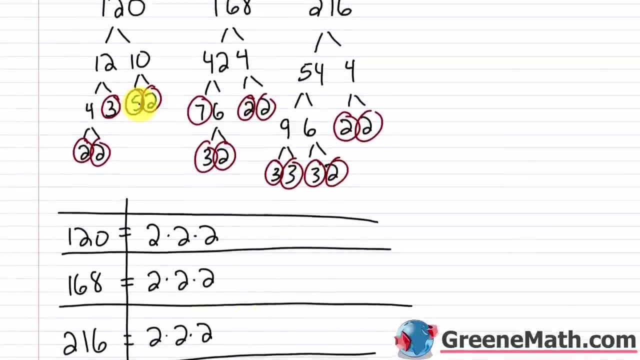 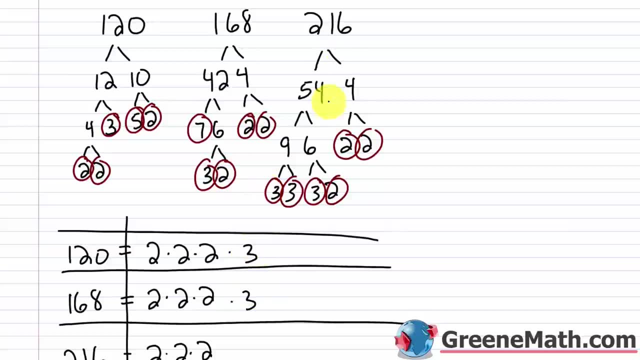 So 2 times, 2 times 2.. And then, kind of going back to 120, I have 1 factor of 3.. So 1 factor of 3.. In 168, I have 1 factor of 3.. In 216, I have 1,, 2,. 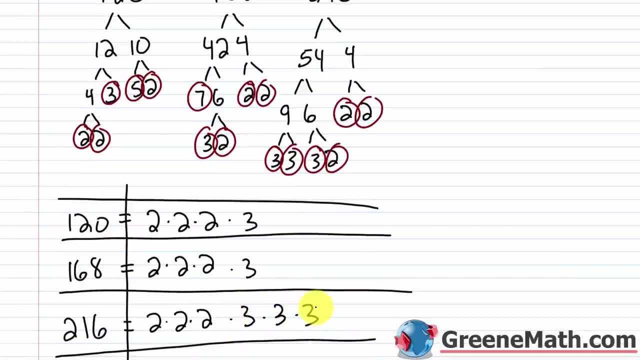 3 factors of 3.. So 1,, 2, 3.. So what I'm going to do to make this obvious? I'm going to mark out what we're missing. Only 1 factor of 3 is common to everything. 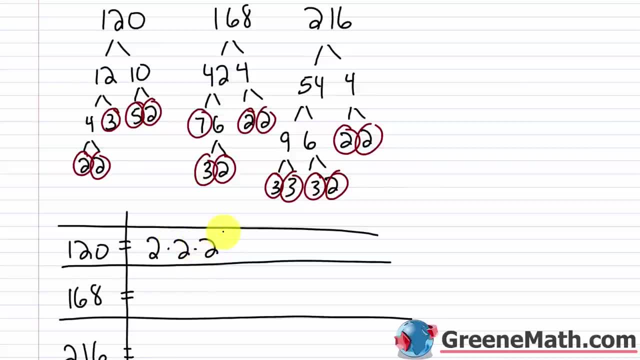 2 times 2 times 2. And let me kind of look at 168 now. So I have 2 times 2 times 2. So I have three factors of 2 there as well. And then at 216, I have three factors of 2 as well. So 2 times 2 times 2. 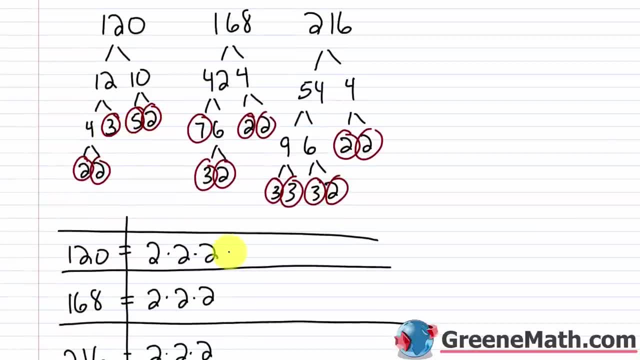 And then kind of going back to 120, I have one factor of 3. So one factor of 3. And 168, I have one factor of 3. 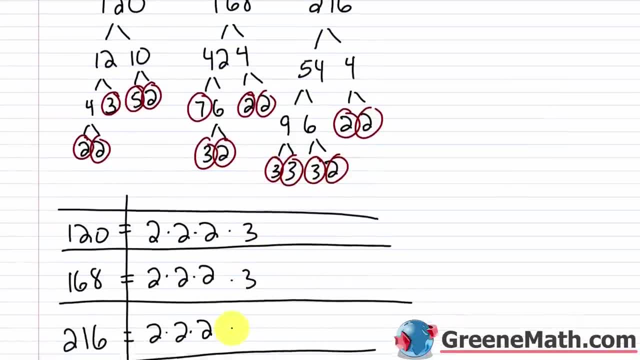 And 216, I have one, two, three factors of 3. So one, two, three. 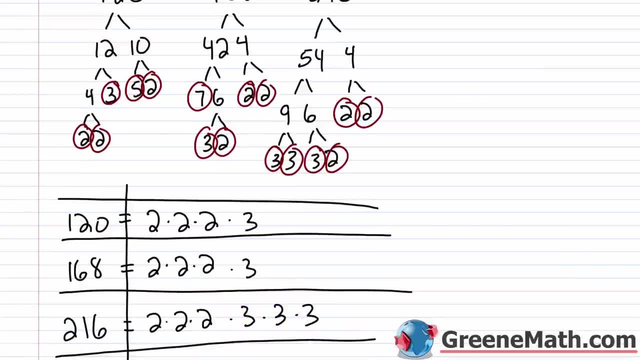 So what I'm going to do to make this obvious, I'm going to mark out what we're missing. All right. Only one factor of 3 is common to everything. Now, moving on, I have a factor of 5 and 120. And then I'm done. 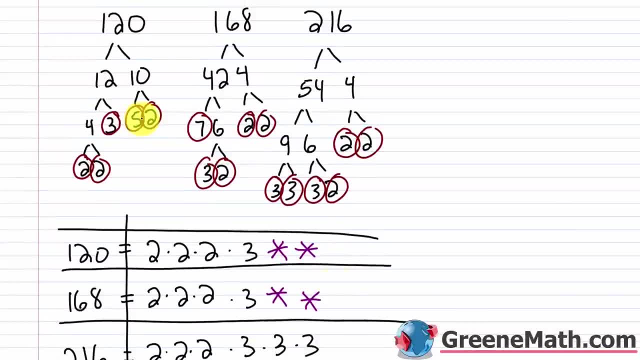 So this one's closed out. I'm just going to put a little x next to it. 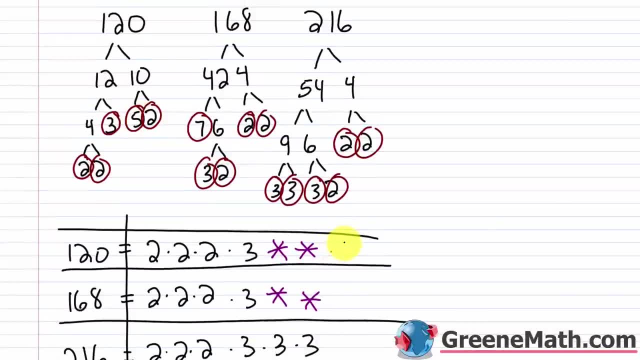 Now moving on. I have a factor of 5 in 120 and then I'm done. So this one's closed out. I'm just going to put a little x next to it. So for 168 I don't have a factor of 5.. 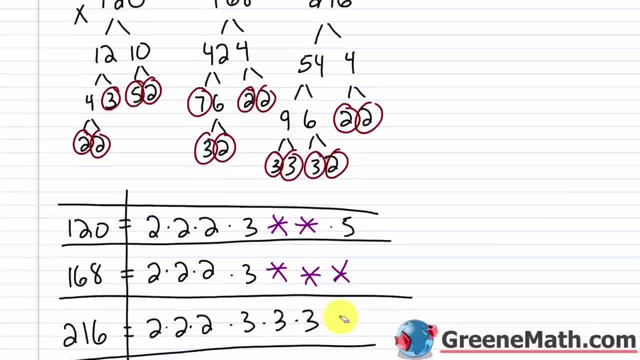 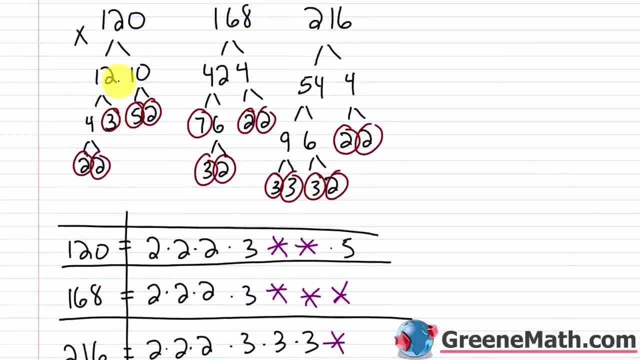 So let me just kind of notate that with this In 116, I also don't have a factor of 5. And then I could stop here if I wanted to, Because once I've closed one of them out, that means anything that appears. 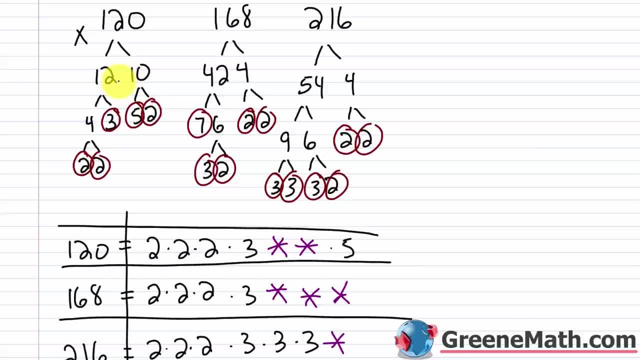 in the other prime factorizations won't matter, because it's not in one of them and it's got to be common in everything. But just for the sake of completeness, in 168 I have a factor of 7. So let me write that. 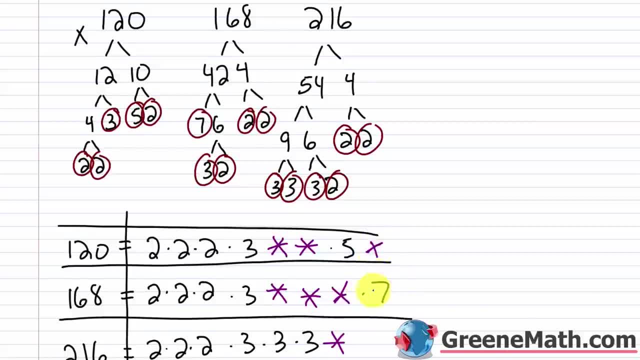 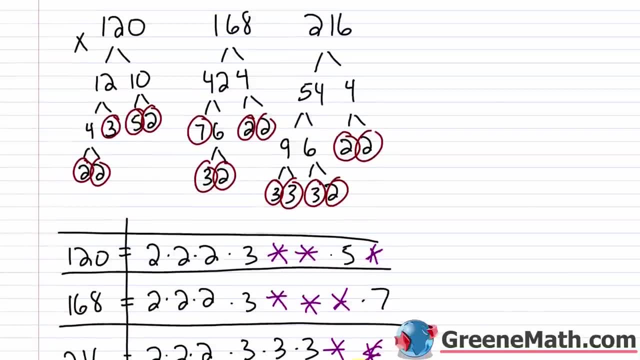 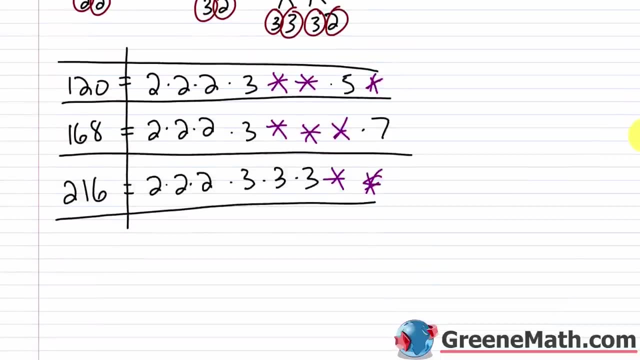 Let me kind of mark this out over here And in 216 I don't have anything else to put in, So let me just put that these are closed out as well. Let me kind of scroll down and get a little more room going. 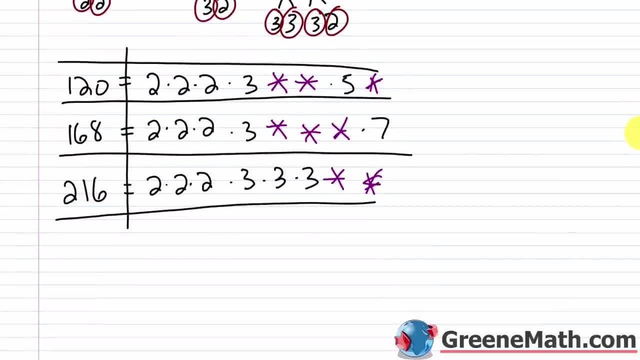 Alright. so again, it's completely obvious what the list is going to be with the way that I've written this table, And if you're struggling with this kind of concept of the GCF, you might want to take the extra time to kind of 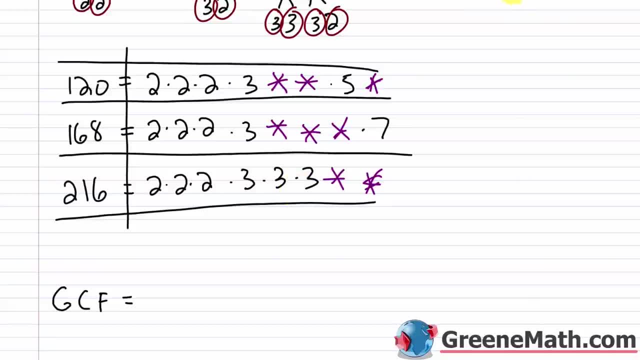 spread everything out and look at what's common. So I know that everything has one, two, three factors of two. So two times two times two is eight. I could write it as two times two times two, or I can just put eight. 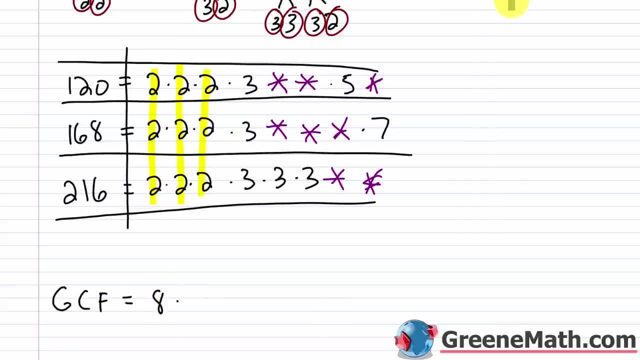 And times. The next thing that's common to everything is going to be a three. I have one factor of three that's common to everything. Now here's where students get confused. They see two additional factors of three down here. That's not common. 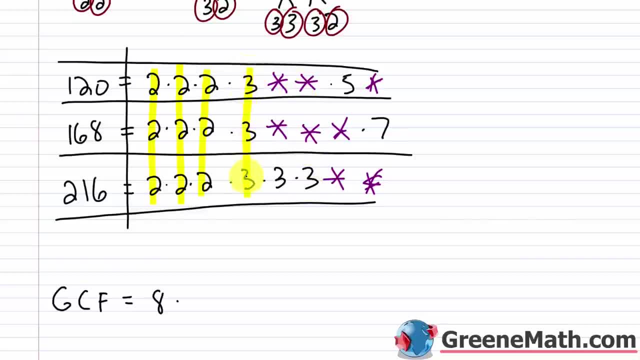 to everything, so you can't put it in. It's got to be common to everything, So I'm going to put times three. Five is not common to everything and seven is not common to everything. This is what's common to everything. It's eight times three. 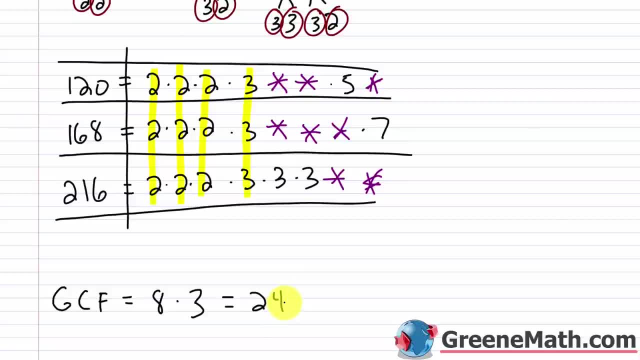 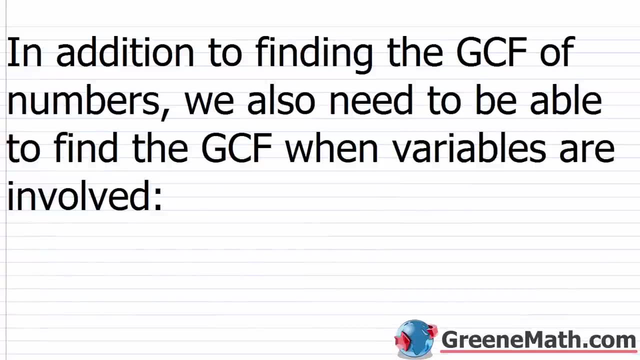 and that is twenty-four, And so that is your greatest common factor for the numbers 120,, 168, and 260.. So hopefully those last two examples gave you a general understanding of how to find the greatest common factor If you need more practice with. 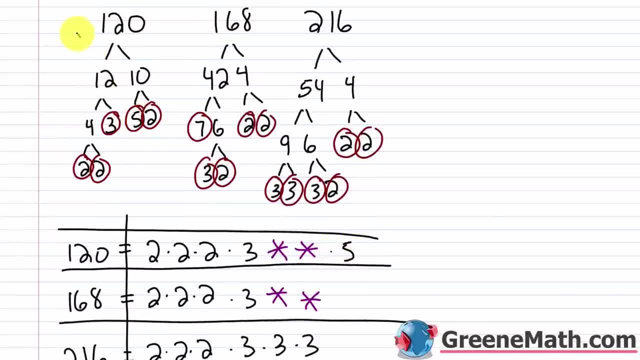 So for 168, I don't have a factor of 5. So let me just kind of look at that. And then I'm going to put a little x next to it. So let me just kind of look at that. So let me just kind of notate that with this. 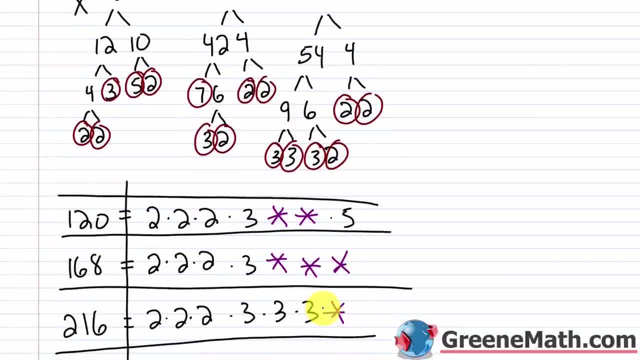 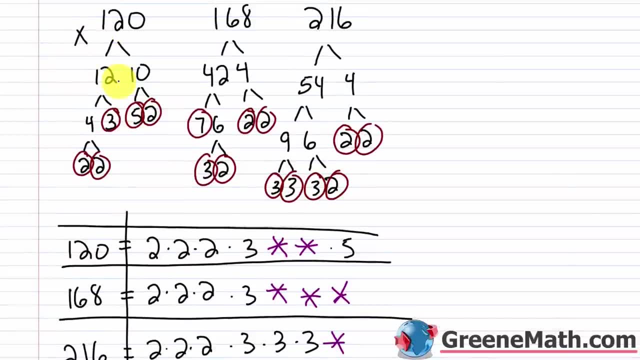 And then 216, I also don't have a factor of 5. And then I could stop here if I wanted to. Because once I've closed one of them out, That means anything that appears in the other prime factorizations won't matter because it's not in one of them. 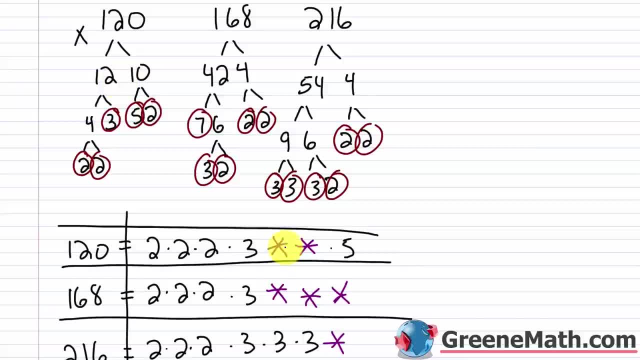 And it's got to be common to everything. But just for the sake of completeness, In 168, I have a factor of 7. So let me write that. Let me kind of mark this out over here. 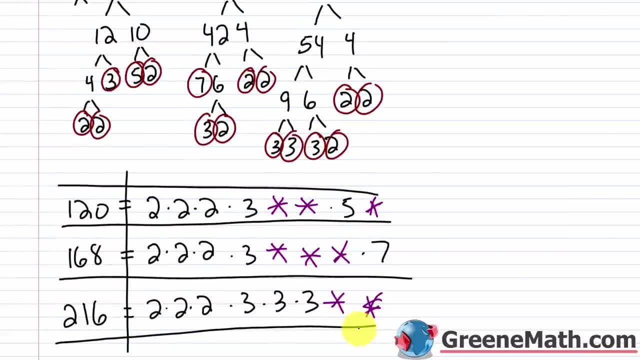 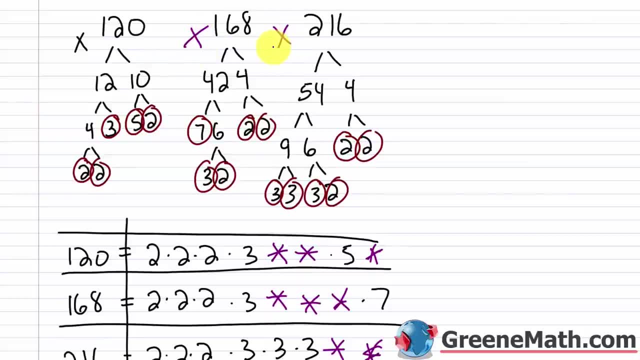 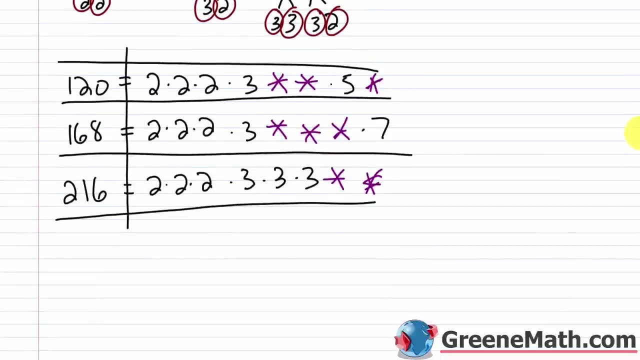 and in 216 i don't have anything else to put in so let me just put that these are closed out as well let me kind of scroll down and get a little more room going all right so again it's completely obvious what the list is going to be right with the way that i've written this table and if you're struggling with this kind of concept of the gcf you might want to take the extra time to kind of 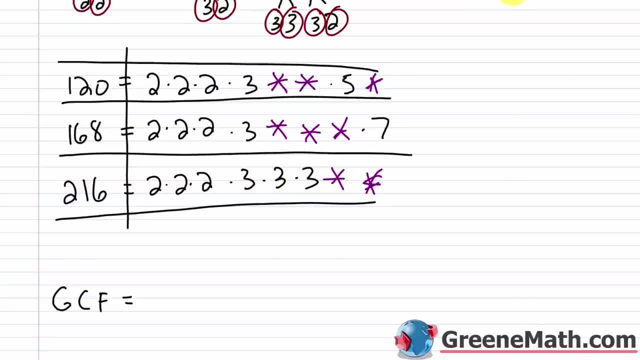 spread everything out and look at what's common so i know that everything has one two three factors of two so two times two times two is eight i could write it as two times two times two right and just put eight and times the next thing that's common to everything is going to be a three right i have one factor of three that's common to everything now here's where students get confused they see two additional factors of three down here that's not common to every of them 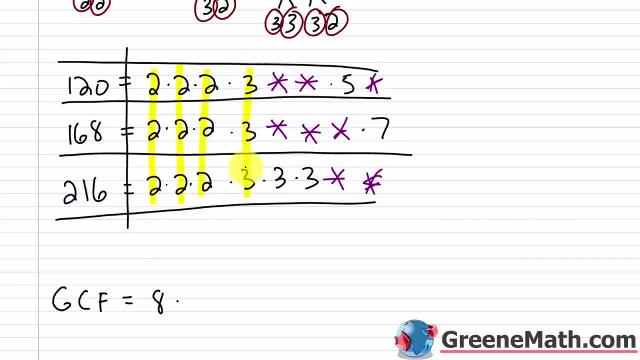 everything. So you can't put it in. It's got to be common to everything. So I'm going to put times three. Five is not common to everything, and seven's not common to everything. This is what's common to everything. It's eight times three, and that is 24. And so that is your greatest common factor for the numbers 120, 168, and 260. So hopefully those last two examples gave you a 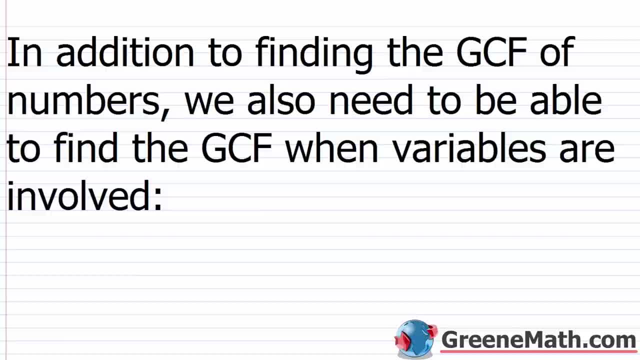 general understanding of how to find the greatest common factor. If you need more practice with this, go back into the pre-algebra lessons and take a look at the video that we made on finding the greatest common factor. Again, this is also called finding the greatest common divisor. 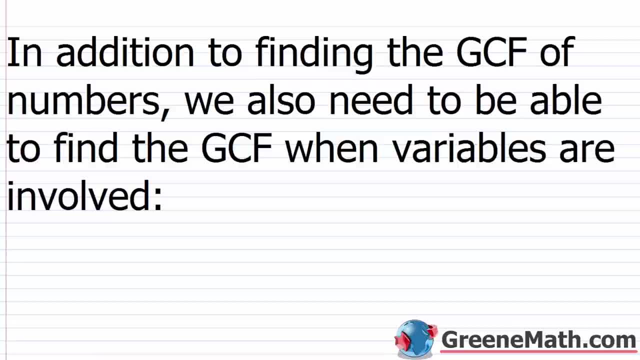 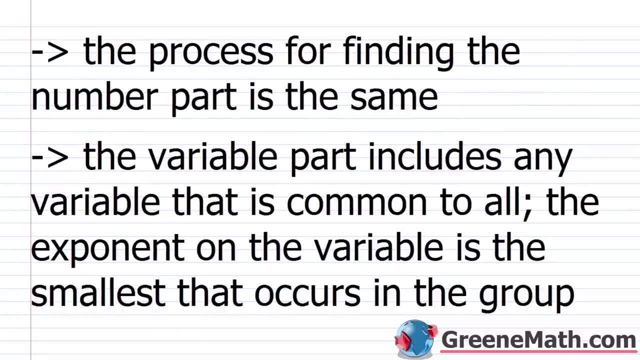 But kind of moving forward and thinking about how we're going to use this for algebra, in addition to finding the GCF, and again that's greatest common factor, of numbers, we also need to be able to find the GCF when variables are involved. Now the process for finding the number part is the same. 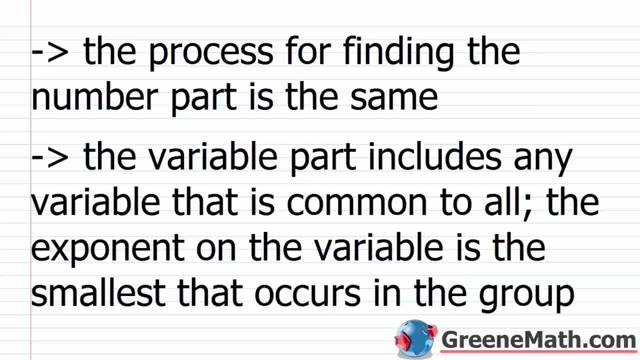 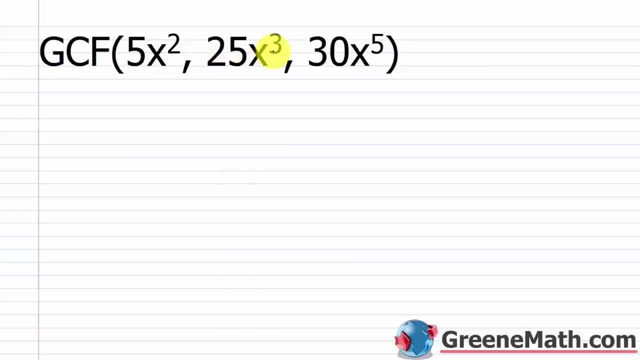 The variable part is a little bit different because you don't need to sit there and make a factor tree. I know you don't need to do that every time for numbers, but when they get kind of big, you really kind of do need to do that. So the variable part just includes any variable that is common to all. The exponent on the variable is the smallest that occurs in the group. So for example, let's look at the greatest common factor for 5x squared, 25x cubed, and 30x to the fifth power. So what am I looking at? Well, I'm going to think about the number parts. I have a 5, I have a 25, and I have a 30. I don't need to go through and factor that. We all should be able to see at this point that the greatest common factor would be 5. 5 doesn't factor. It's a prime number. 25 is what? It's two factors of 5. 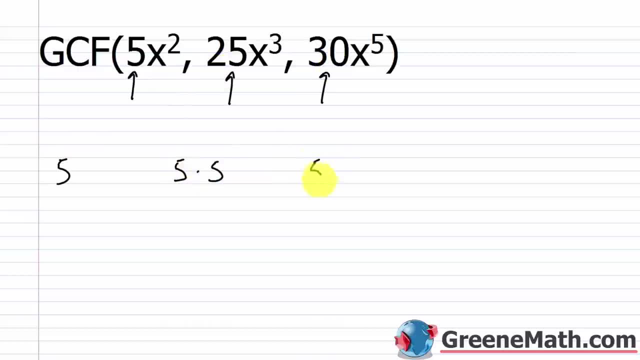 It's 5 times 5. And then 30 is going to be 5 times 6, or 5 times 2 times 3. So if I look at these, what's common to everything? It's just a 5, right? 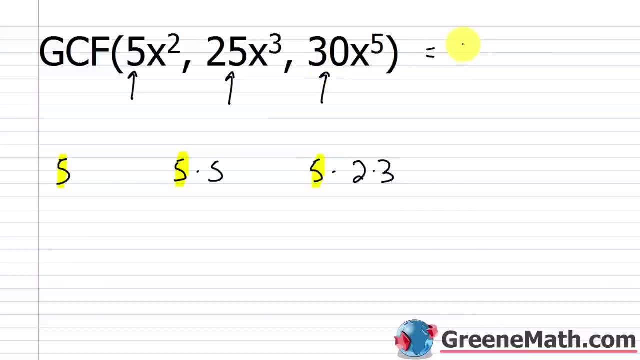 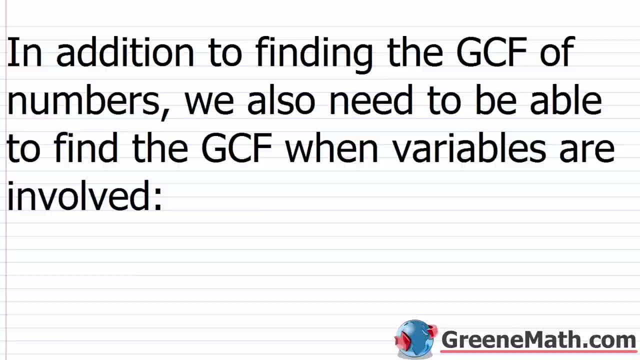 this. go back into the pre-algebra lessons and take a look at the video that we made on finding the greatest common factor. Again, this is also called finding the greatest common divisor, But kind of moving forward and thinking about how we're going to use this for algebra. 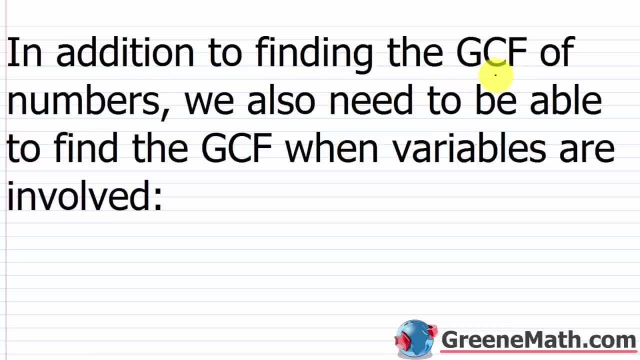 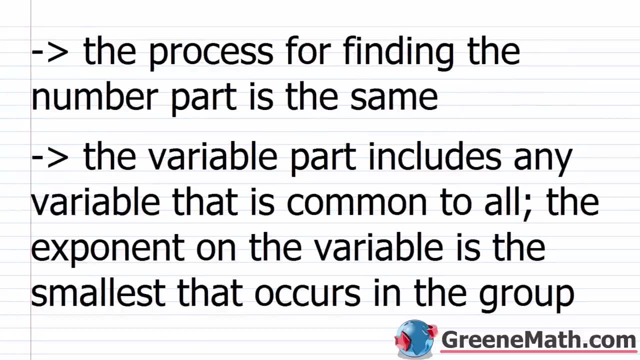 in addition to finding the GCF- and again that's greatest common factor of numbers- we also need to be able to find the GCF when variables are involved. Now the process for finding the number part is the same. The variable part is a little bit different. 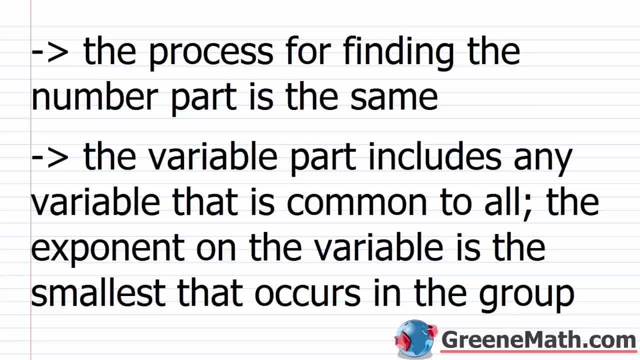 because you don't need to sit there and make a factor tree. I know you don't need to do that every time for numbers, but when they get kind of big you really kind of do need to do that. So the variable part just includes any variable. 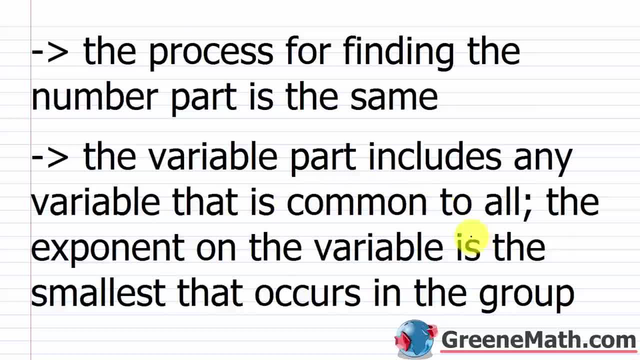 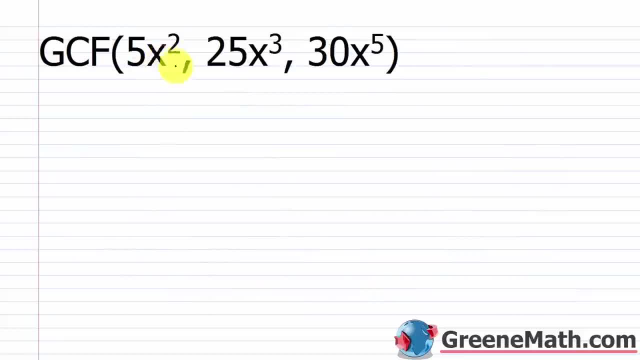 that is common to all. The exponent on the variable is the smallest that occurs in the group. So, for example, let's look at the greatest common factor for 5x squared, 25x cubed and 30x to the fifth power. 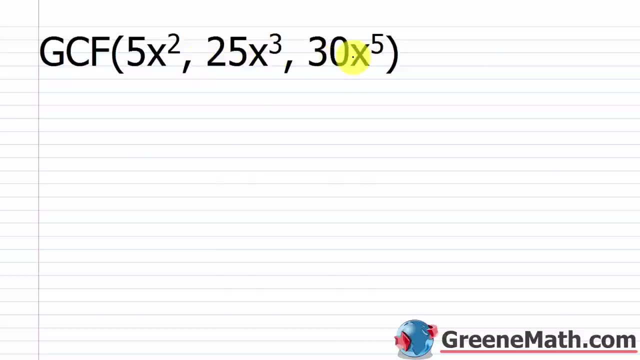 So what am I looking at here? Well, I'm going to think about the number parts. I have a 5,, I have a 25, and I have a 30. I don't need to go through and factor that. We all should be able to see at this. 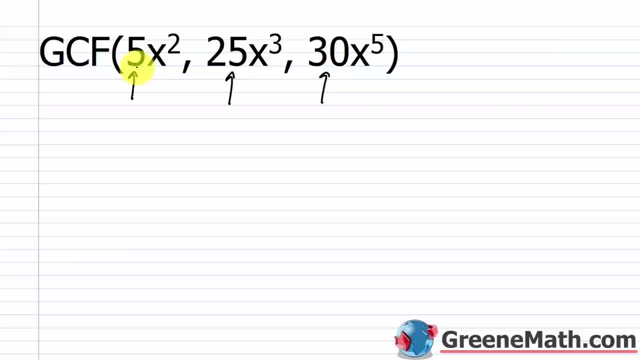 point that the greatest common factor would be 5.. 5 doesn't factor, It's a prime number. 25 is what It's, two factors of 5. It's 5 times 5.. And then 30 is going to be 5 times 6,. 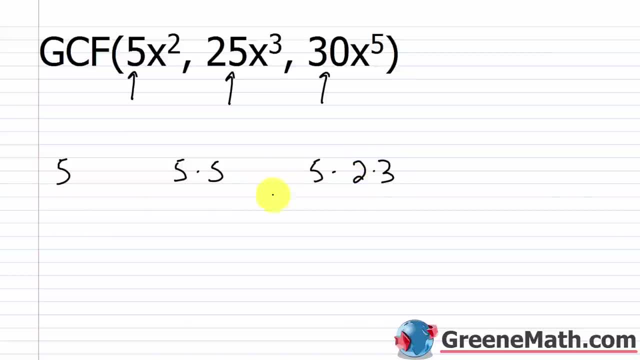 or 5 times 2 times 3.. So if I look at these, what's common to everything? It's just a 5.. Right, So I can eyeball that and see that the number part here is going to be 5.. But what's? 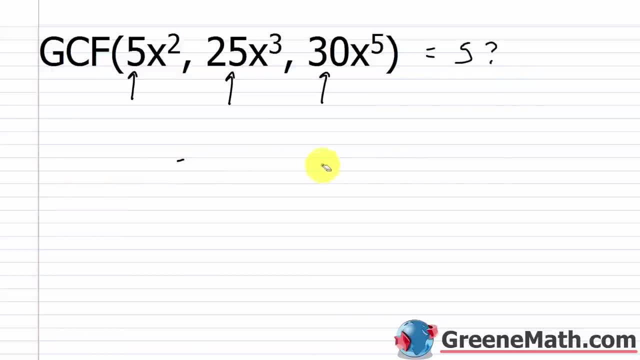 the variable part. Well, all I do is look at what's common to everything here. I have x squared, I have x cubed and I have x to the fifth power. What is x squared? It's x times x. What is x cubed? 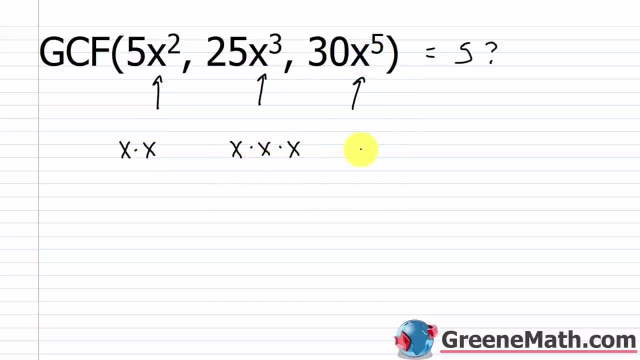 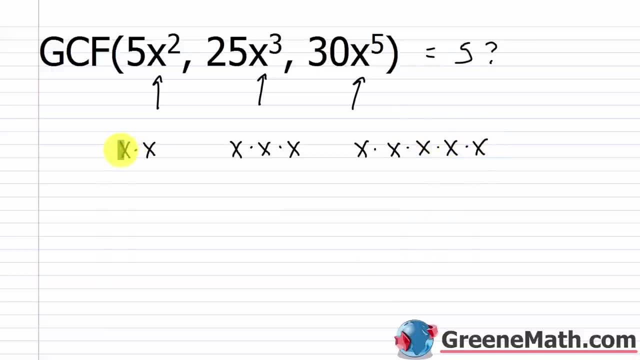 So what's common to everything? Well, since I only have two factors of x here, that's as many factors that's going to be common to everything. I have 2 here. I have 3 here, but only 2 would be in common with this. I have 5 here, but again, only 2 would be in common with this. So in other words, all I need to do is look for the smallest exponent that appears on that variable that is 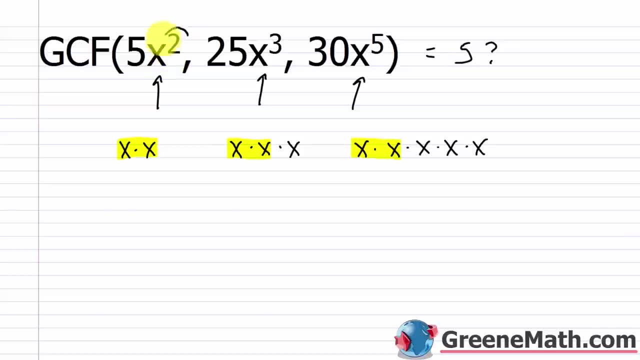 common to all. The smallest exponent occurs right here. It's a 2. So I just use that when I build my VCF. So this is basically just going to be 5x squared. That's going to be my greatest common 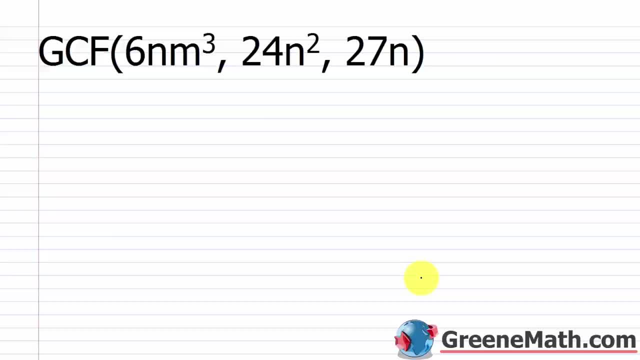 factor. All right, for the greatest common factor of 6nm cubed, 24n squared, and 27n, again, let's think about the number parts first. So can we eyeball this and do it? I can. Maybe you're not 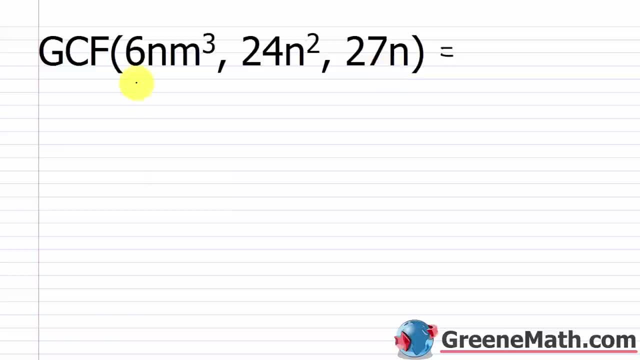 at that level yet, but very quickly you will be. I know right away that 27 is only going to have 3. 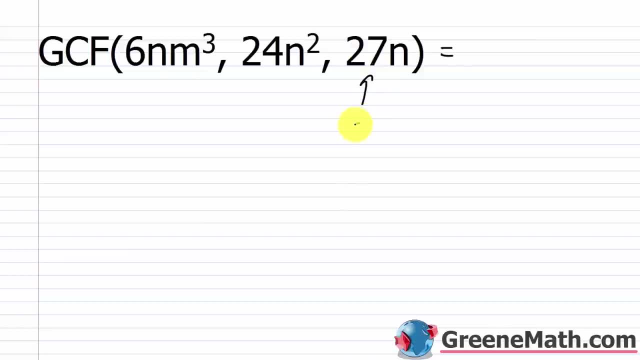 For 24, it's divisible by 3. 24 divided by 3 is what? It's 8. This is 8 times 3. And I could sit there and write it as 2 cubed times 3. But again, I don't need to do that at this point. For 6, I know that's 2 times 3. If I look at this, what's going to be common to everything? It's not going to be 2 because there's no 2 in the prime factorization of 27. So I can just not think about that. 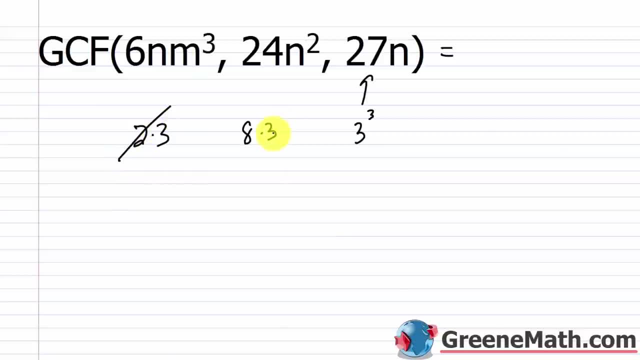 It's only going to be 3. This has a factor of 3. This has a factor of 3. And this has three factors of 3. But what's going to be common is only one of those. So the number part is just going to be a 3. Now, when we get to the variable part, again, if I think about this, you first ask the question, is that variable common to everything? So I have an n here. I have an n squared here and an n here. So the answer to that is yes. 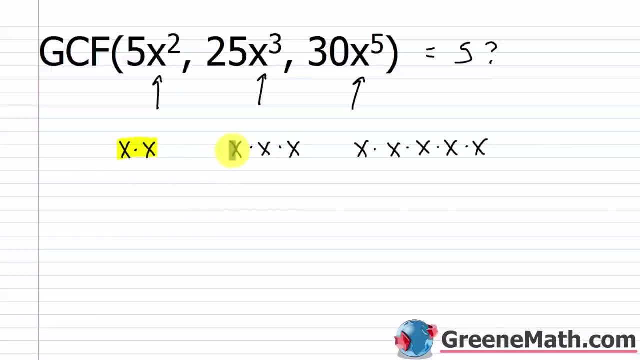 factors. that's going to be common to everything. I have 2 here, I have 3 here, but only 2 would be in common with this. I have 5 here, but again, only 2 would be in common with this. So, in other words, 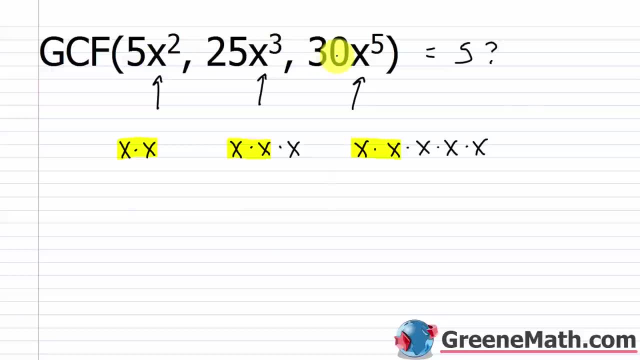 all I need to do is look for the smallest exponent that appears on that variable. that is common to all. The smallest exponent occurs right here: It's a 2. So I just use that when I build my GCF. So this is basically. 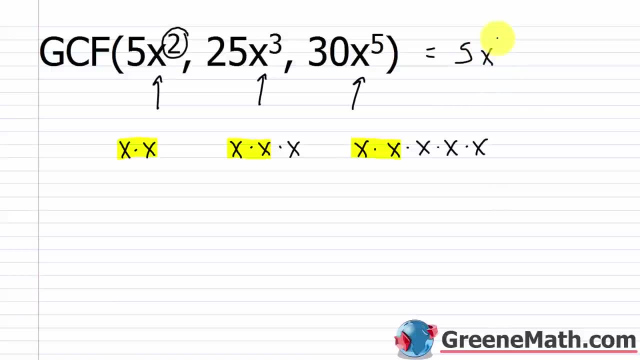 just going to be 5 x squared. That's going to be my greatest common factor. Alright, for the greatest common factor of 6 n m cubed, 24 n squared and 27 n. Again, let's think about the. 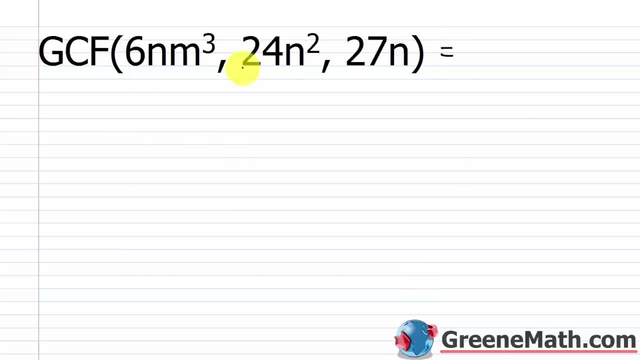 number parts first. So can we eyeball this and do it? I can. Maybe you're not at that level yet, but very quickly you will be. I know right away that 27 is only going to have 3 as a prime factor. right, It's 3 cubed. 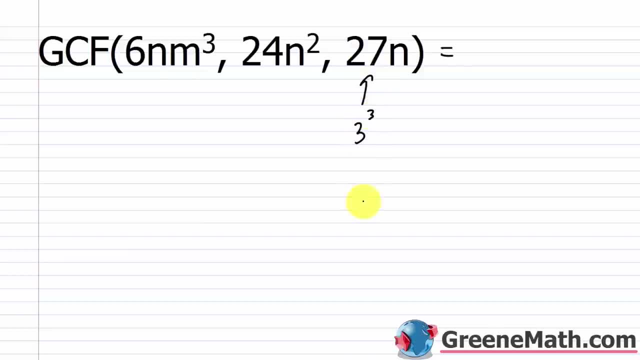 This right here is 3 cubed For 24, it's divisible by 3.. 24 divided by 3 is what It's 8.. This is 8 times 3. And I can sit there and write it as 2 cubed. 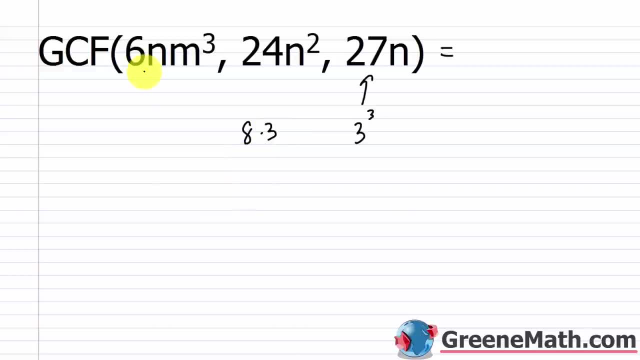 times 3.. But again, I don't need to do that at this point- For 6, I know that's 2 times 3.. If I look at this, what's going to be common to everything? It's not going to be 2. 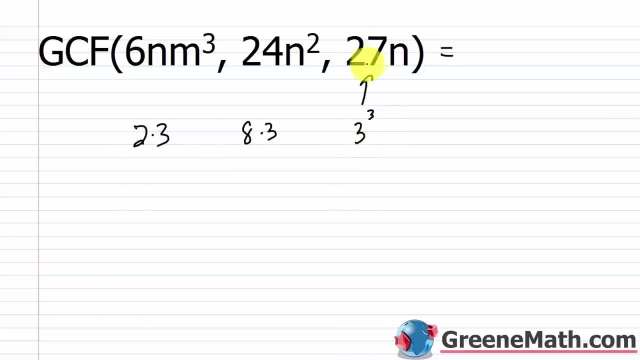 because there's no 2 in the prime factorization of 27.. So I can just not think about that. It's only going to be 3.. This has a factor of 3,, this has a factor of 3, and this has 3 factors. 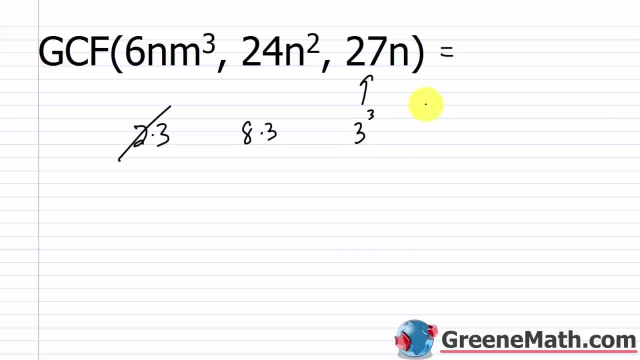 of 3, but what's going to be common is only one of those, So the number part is just going to be a 3.. Now, when we get to the variable part again, if I think about this, you first ask the question is that: 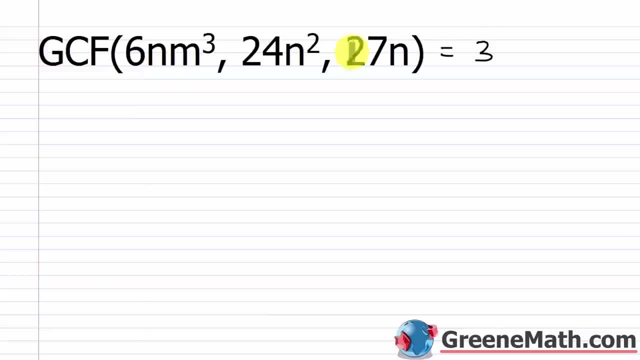 variable common to everything. So I have an n here, I have an n squared here and an n here. So the answer to that is yes. Then what's the smallest exponent that occurs in that group? Well, here I have n to the first power, n squared. 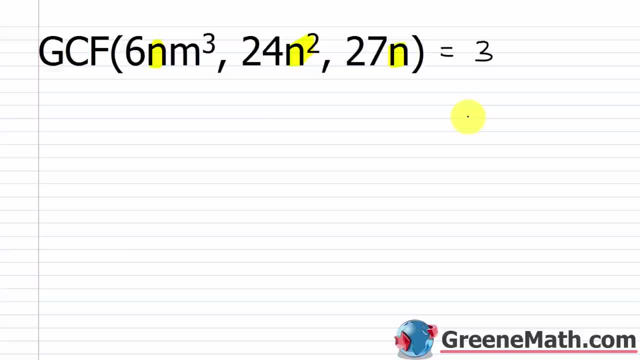 What's the smallest exponent that occurs in that group? Well, here I have n to the first power, n squared, and n to the first power. So an exponent of 1 would be the smallest, right? So n to the first power, or just n, would go into the GCF. Now, I have an m cubed here, but I don't have an m here or here. It's got to be common to everything. And so there's not going to be a variable m that's going to go into this. So your GCF is just going to be n to the first power. And so I have going to be 3n. All right, let's take a look at another one. So we have the greatest common 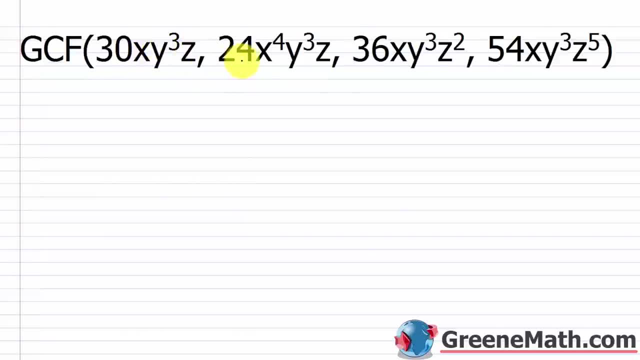 factor of 30xy cubed z, 24x to the fourth y cubed z, 36xy cubed z squared, and 54xy cubed z to the fifth. So what is the GCF? So let's think about the number part first. So we have a 30. Let's think about that. So that's 3 times 10. 10 is 5 times 2. 3 times 5 times 2. 24. 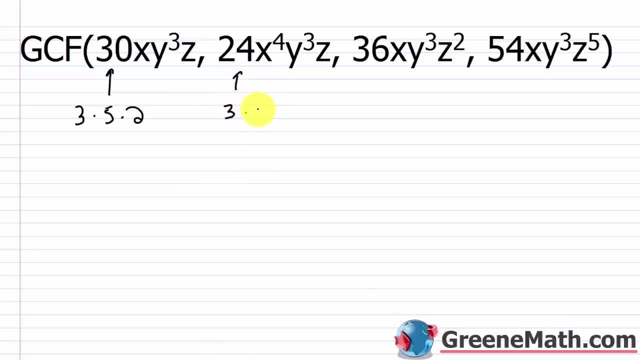 Let's think about that as 3 times... All I have is a 2 here. So 3 times 2 would be 6, and then times another 4, and then 36. Let's do... Again, all I have is a 2 here. So let's do 2 times 18. 18 would be 9. All I have is a 3 here. So let's do 2 times 3. So that's 6. So 2 times 3 times 6. And I'm breaking this down to where I already know that all I'm going to have is a 3 times a 2 that's common to everything, right? So I can already see from these first few that the GCF is going to be a 6 in terms of the number part, right? Because this guy right here, if you think about it, is really what? It's 6 times 9. So if I look at this, nothing has a 5 in the prime factorization other than 30. So you can just mark that out. So all I have here really is just 3 times 2 or 6. So I'm just looking for that in everything else, and it hasn't. This has a 6, this has a 3 times 2 or 6, this has 3 times 2 or 6, and then this has a 6. So the GCF, the number part at least, is going to be 6. Now what about the variable part? What about the variable part? Well, is X common to everything? I have an X here, here, here, and here. So let me put an X in there. 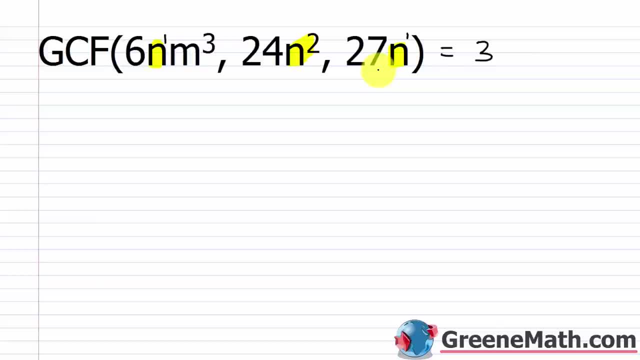 and n to the first power. So an exponent of 1 would be the smallest, So n to the first power or just n would go into the GCF. Now I have an m cubed here, but I don't have an m here or here. 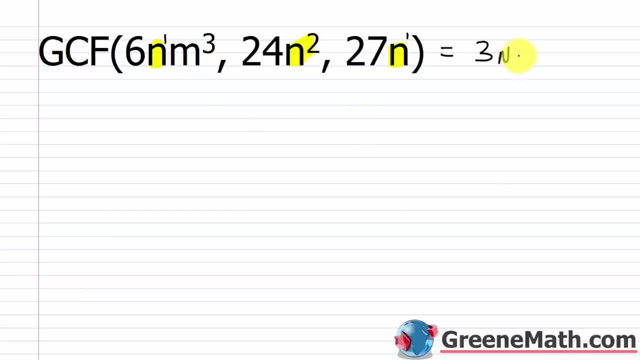 It's got to be common to everything, And so there's not going to be a variable m that's going to go into this. So your GCF is just going to be 3n. Alright, let's take a look at another one. 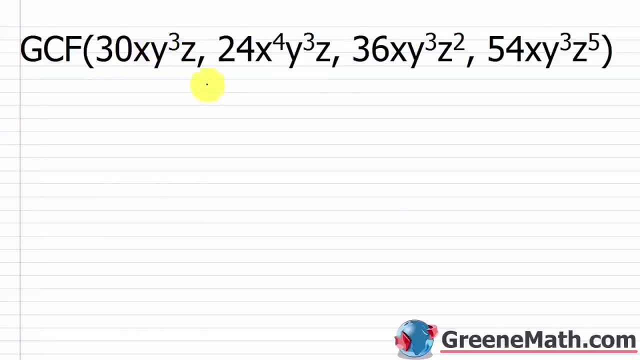 So we have the greatest common factor of the GCF, which is 30xy cubed z, 24x to the fourth, y cubed z, 36xy cubed z, squared, and 54xy cubed z to the fifth. 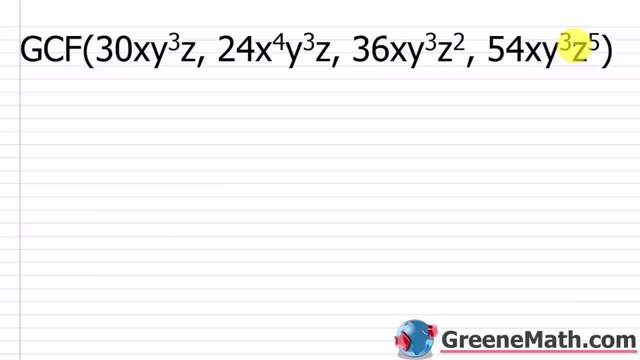 So what is the GCF? So let's think about the number part first. So we have a 30. Let's think about that. So that's 3 times 10.. 10 is 5 times 2.. 3 times 5 times 2.. 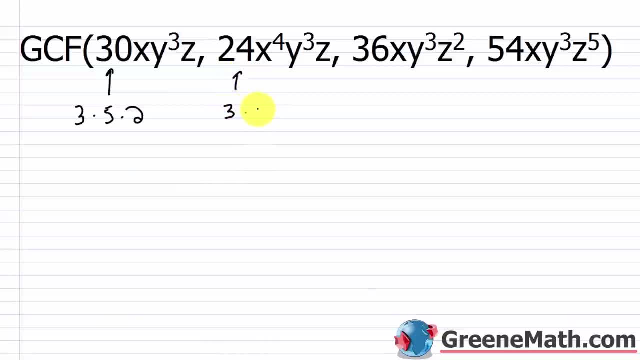 24.. Let's think about that as 3 times. all I have is a 2 here, so that would be 6.. And then times another 4.. And then 36.. Let's do again. all I have is a 2 here. 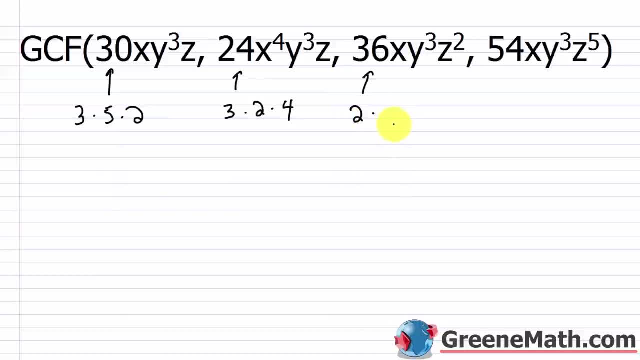 So let's do 2 times 18.. 18 would be 9.. All I have is a 3 here. So let's do 2 times 3.. So that's 6.. So 2 times 3 times 6.. 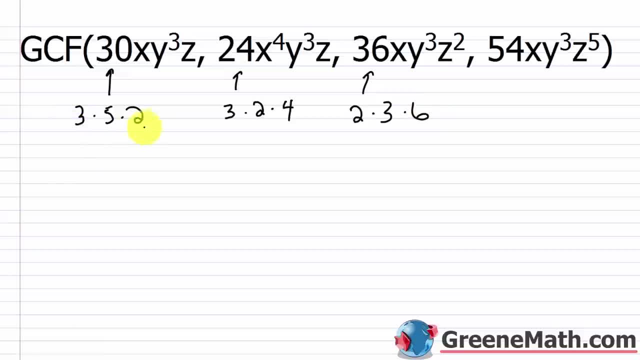 And I'm breaking this down to where I already know that all I'm going to have is a 3 times a 2. that's common to everything, Right? So I can already see from these first few that the GCF is going to be. 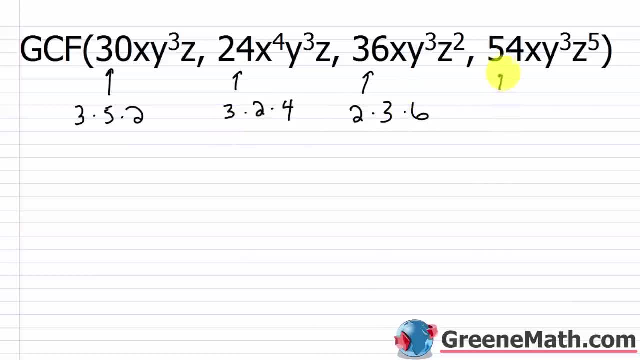 a 6 in terms of the number part Right, Because this guy right here, if you think about it, is really what It's: 6 times 9.. So, if I look at this, nothing has a 5 in the prime factorization. 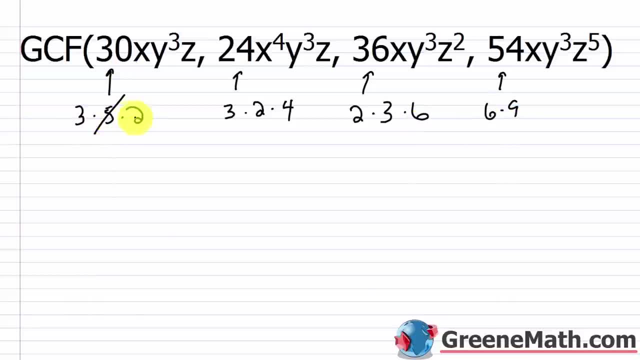 other than 30. So you can just mark that out. So all I have here really is just 3 times 2 or 6. So I'm just looking for that in everything else and it hasn't. This has a 6.. This has a 3 times 2 or 6.. 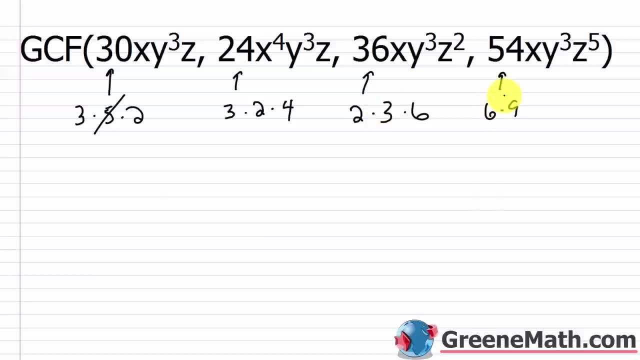 This has 3 times 2 or 6. And then this has a 6. So the GCF, the number part at least, is going to be 6.. Now, what about the variable part? What about the variable part? Well, is x common to everything? 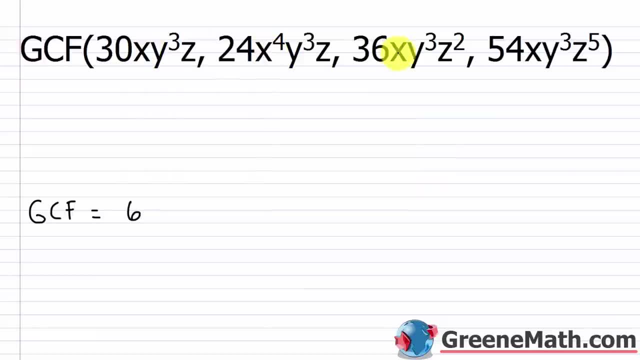 I have an x here, here, here and here, So let me put an x in there. Now, what's the exponent going to be? Again, you look for the smallest one, So this is the number 1,, 4,, 1,. 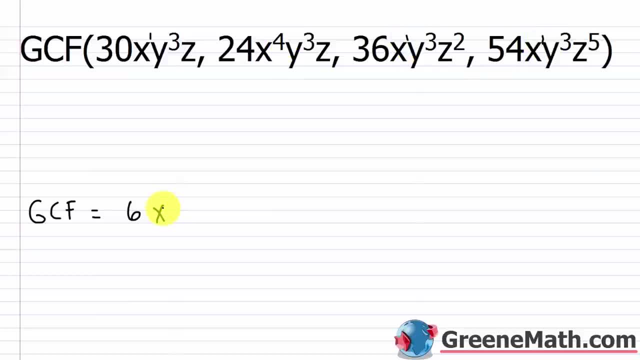 and 1.. So it's just going to be to the first power, or just x. Now the next variable. we have y cubed, So y cubed, y cubed, y cubed and y cubed, So everything is y cubed. 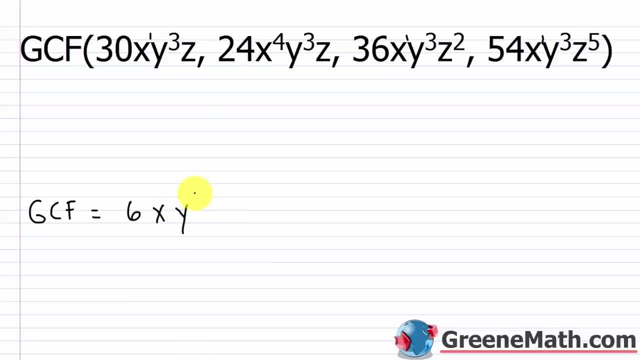 So the smallest exponent is a 3. That's going to go in there. So this is going to be y cubed. And then for the variable z, I have z, z, z squared, and z to the 5th power. 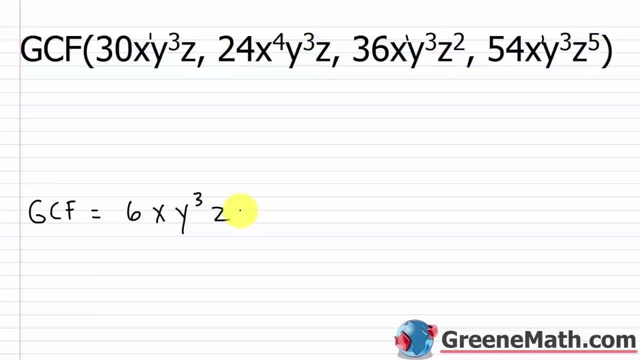 The smallest exponent is a 1.. So I just throw a z in there, And so my greatest common factor is going to be 6xy cubed z. Alright, let's take a look at another one. So we have 32q to the 8th power. 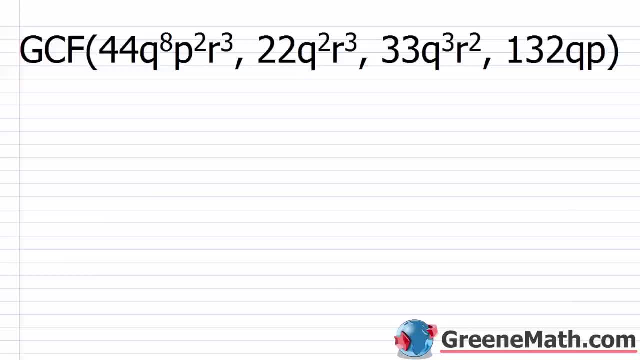 p squared- r cubed, 22q squared r- cubed, 33q cubed, r squared, and then 132qp Again. let's look at the number part, And I think it's obvious, at least to myself, that the GCF for the number part is 11.. 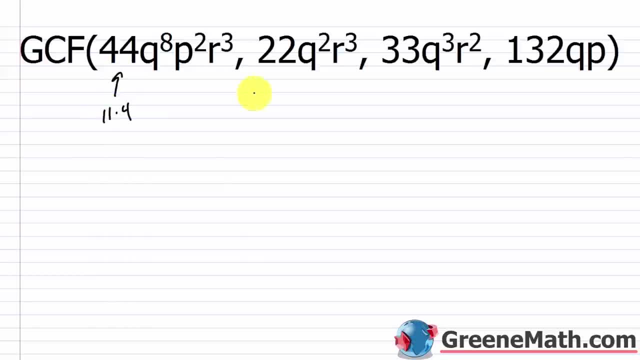 Alright, this is 11 times 4. this is 11 times 2. this is 11 times 3. this is 11 times 12.. And I can eyeball that and see it, And again over time, you're going to be able to do that as well. 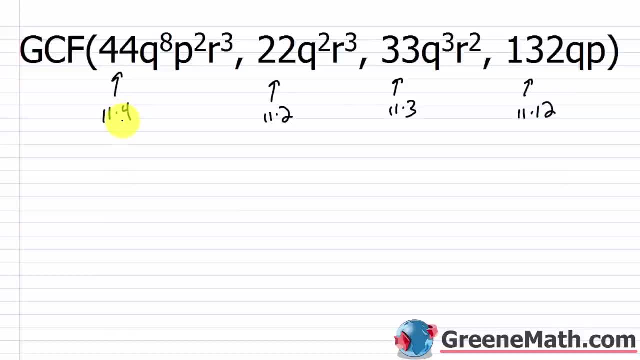 if you can already, And you can easily see that, okay, this has a 4,, that's 2 times 2.. This has 1 factor of 2, but no factors of 2 here, So this isn't going to work. 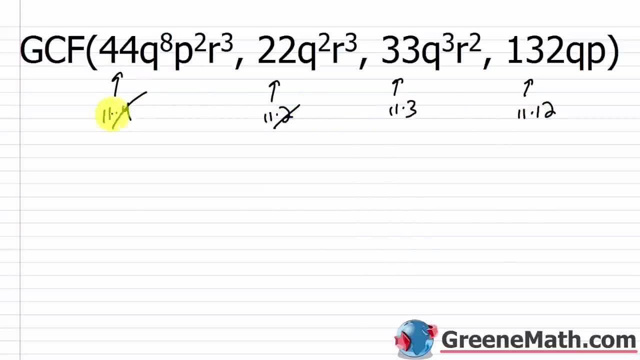 That's not going to work, And nothing else is in these other than 11, so you can just cross these out as well. You're only left with the possibility of 11 for your number part. So let's get rid of this. 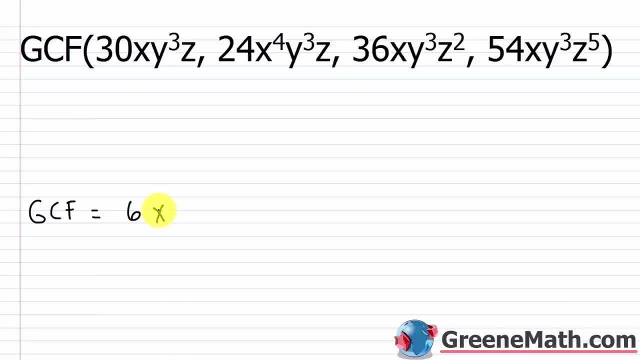 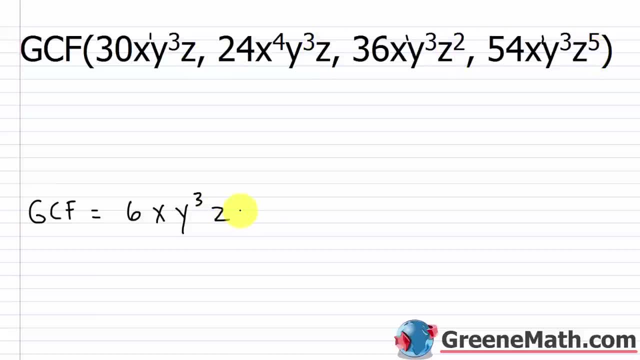 smallest exponent is a 1. So I just throw a Z in there. And so my greatest common factor is going to be 6XY cubed Z. All right, let's take a look at another one. So we have 44Q to the eighth power, 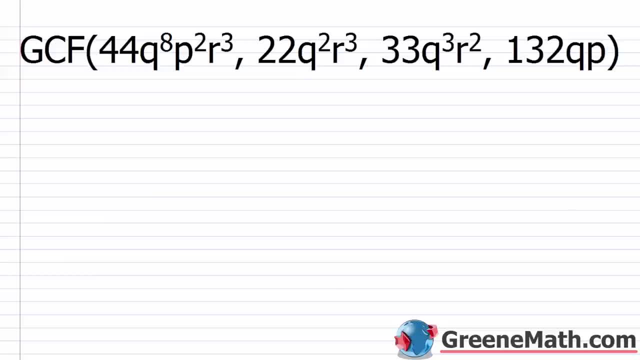 P squared R cubed, 22Q squared R cubed, 33Q cubed R squared, and then 132QP. 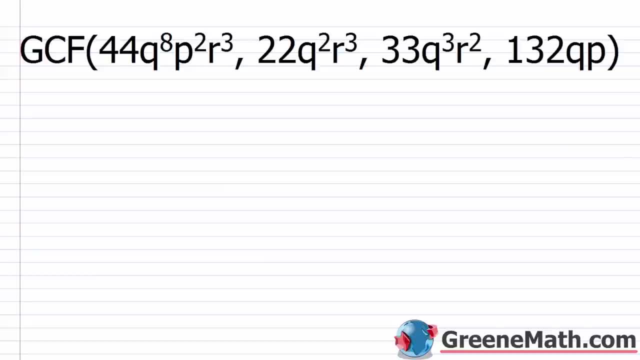 Again, let's look at the number part. And I think it's obvious, at least to myself, that 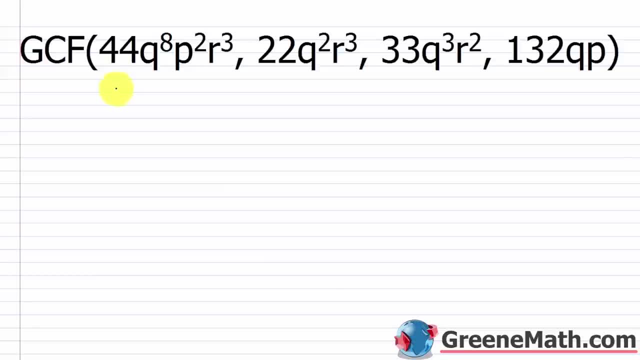 the GCF for the number part is 11, right? This is 11 times 4. This is 11 times 4. This is 11 times 4. This is 11 times 2. This is 11 times 3. This is 11 times 12. All right, I can eyeball that and see. And again, over time, you're going to be able to do that as well if you can already. And you can easily see that, okay, this has a 4. That's 2 times 2. This has one factor of 2, but no factors 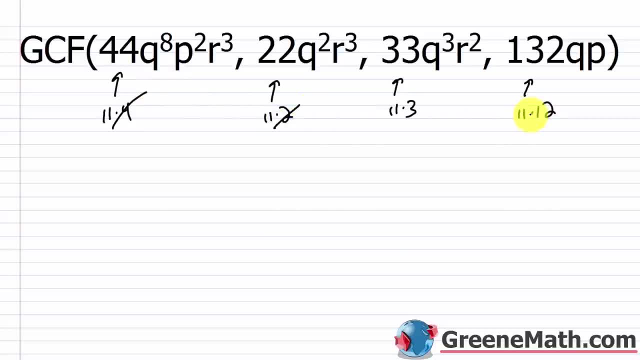 of 2 here. So this isn't going to work. That's not going to work. And nothing else is in these other than 11. So you can just cross these out as well. You're only left with the possibility of 11 for your number part. So let's get rid of this. 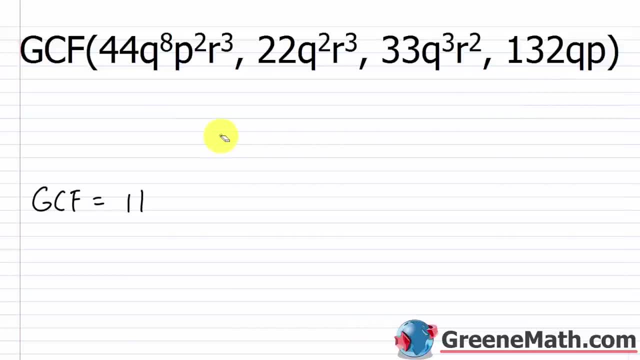 Let's think about what the variable part would be. So I have Q, Q, Q, and Q. The smallest exponent is on this one, right? This is to the first power. You've got cubed, squared, and to the eighth power. 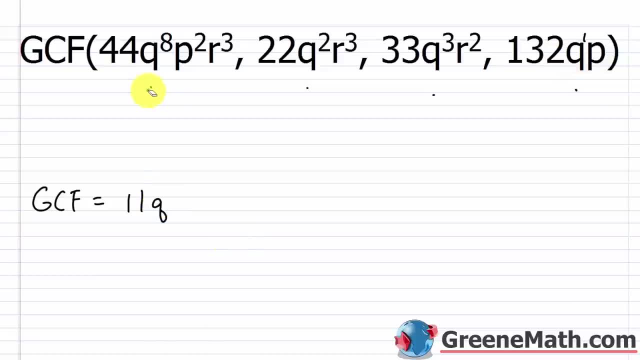 So we're going to go with just Q. Then when I look at the next variable that appears, it's P. So I have P squared, no P here, so you can just stop, right? It doesn't matter that there's a P 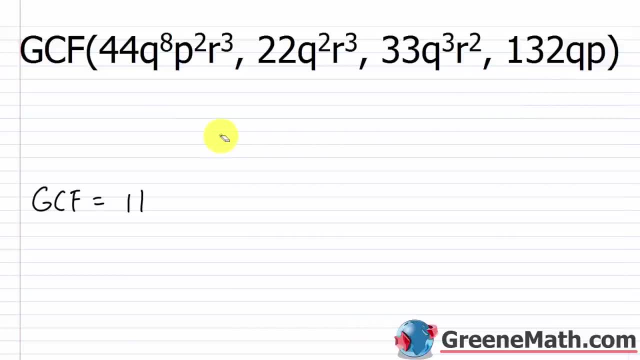 Let's think about what the variable part would be. So I have q, q, q and q. The smallest exponent is on this one. This is to the first power. You've got cubed squared to the eighth power, So we're going to go with. 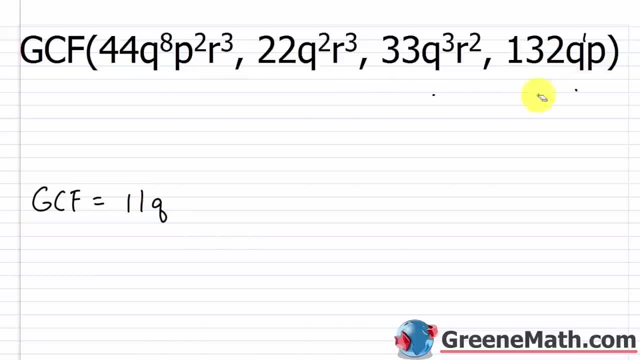 just q. Then when I look at the next variable that appears it's p. So I have p squared. no p here, so you can just stop. It doesn't matter that there's a p down here If it's not common to everything. 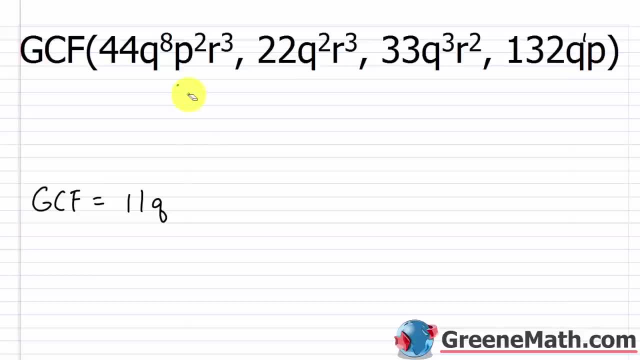 it does not go in. Now the next variable that appears is r So r cubed, r, cubed r squared. no r here, not common to everything, doesn't go in. So your GCF, your greatest common factor here, is just going to be 11q. 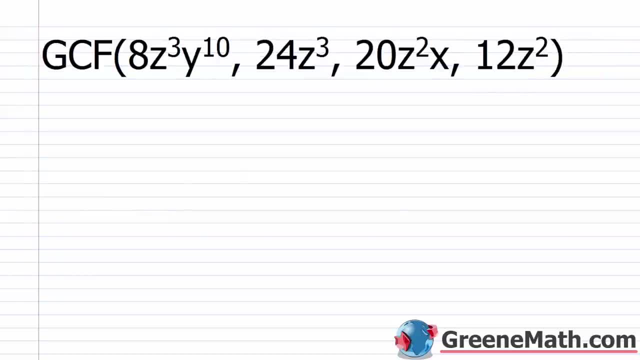 Alright. so let's take a look at 8z cubed y to the 10th, 24z cubed, 20z squared x 12z squared. So for the number part, everything here is divisible by 2.. 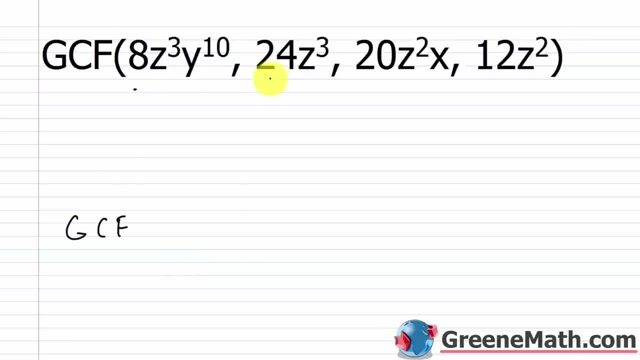 So I kind of think about that in my head: Okay, this is divisible by 2,, this is divisible by 2, so is this? so is this? Everything is also divisible by 4.. So I can think about this as 4 times 2,. 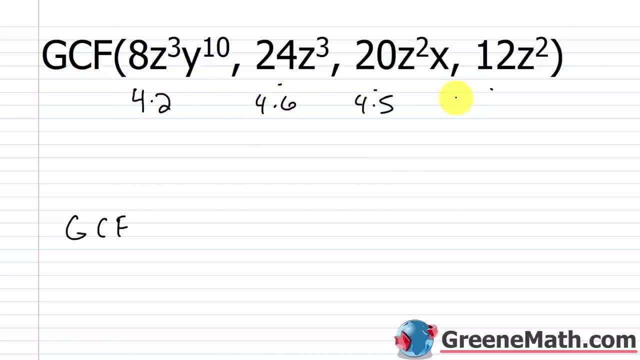 4 times 6,, 4 times 5, and 4 times 3.. Now, because, if I look at this right here, this is a 5, this is a 3.. This is a 2 and this is a 6.. So, if I think about this, 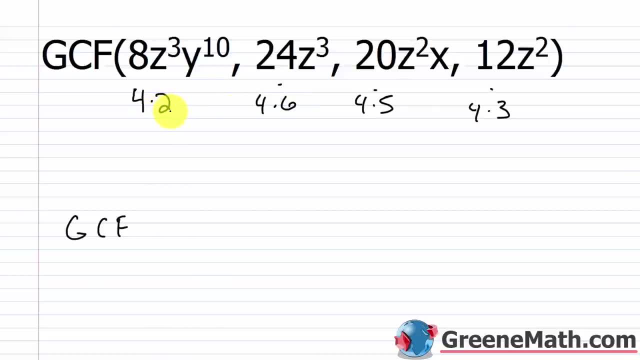 does everything else have another factor of 2? Meaning is it divisible by 8?? The answer is no, So I can mark this out and then basically everything else crumbles right. I can just mark all these out, because the 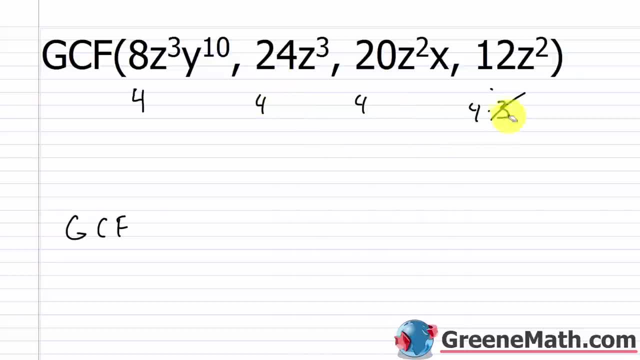 greatest common factor. the number part is just going to be a 4, right, Because it's got to be common to everything. So little tricks like that are going to speed up your work dramatically. So the number part is 4,. 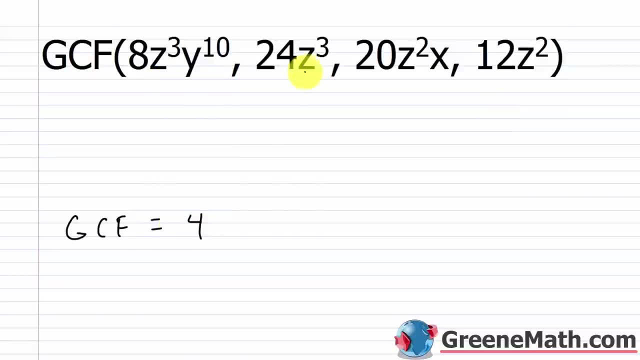 and then for the variable parts, I have z, z, z and z. Smallest exponent is a 2, right: z cubed, z cubed, z squared, z squared, so z squared. and then I have a y to the tenth. 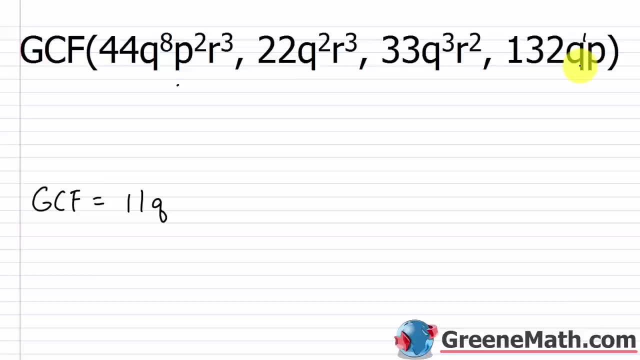 down here. If it's not common to everything, it does not go in. Now the next variable that appears is R. So R cubed, R cubed, R squared, 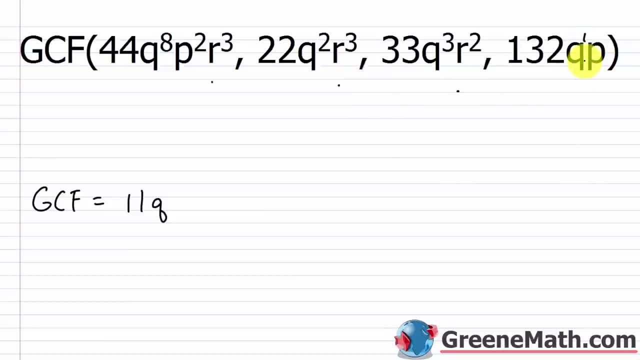 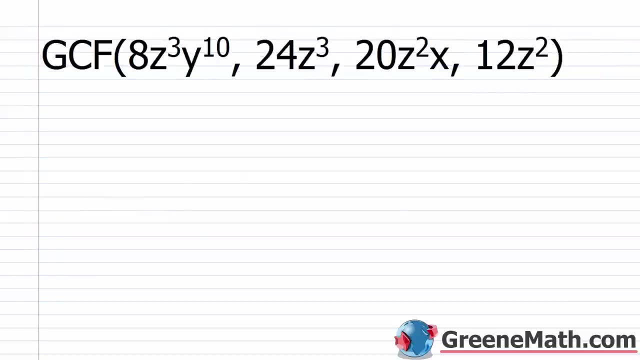 no R here, not common to everything, doesn't go in. So your GCF, your greatest common factor here, is just going to be 11Q. All right, so let's take a look at 8Z cubed, Y to the 10th, 24Z cubed, 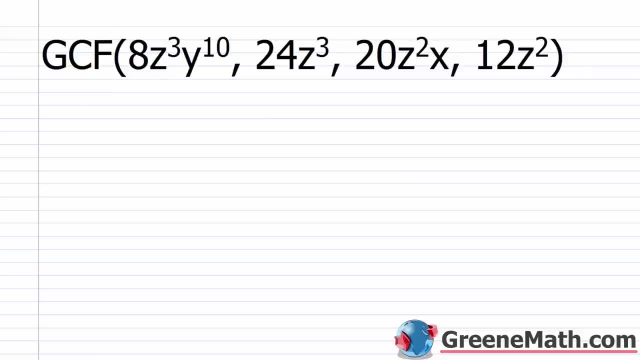 20Z squared X, 12Z squared. So for the number part, for the number part, everything here is divisible by 2. So I kind of think about that in my head. So, okay, this is divisible by 2, this is divisible by 2, so is this, so is this. 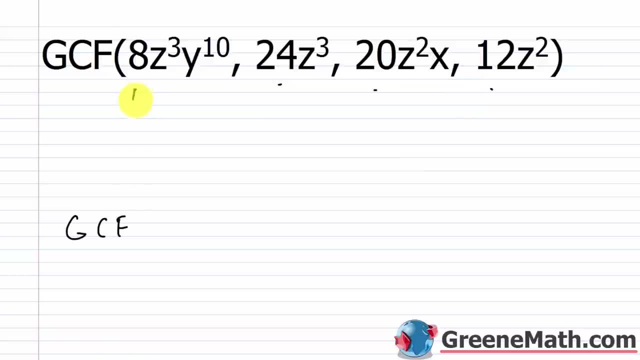 Everything is also divisible by 4. So I can think about this as 4 times 2, 4 times 6, 4 times 5, and 4 times 3. Now, because if I look at this right here, this is a 5, this is a 3, this is a 2, and this is a 6. So if I think about this, does everything else have another factor of 2? 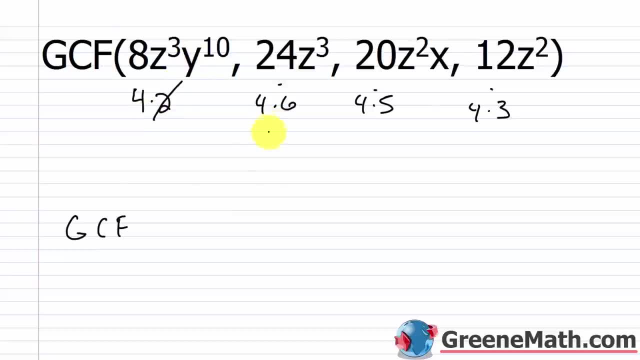 Is it divisible by 8? The answer is no. So I can mark this out, and then basically everything else crumbles, right? I can just mark all these out, because the greatest common factor, the number part, is just going to be a 4, right? Because it's got to be common to everything. So little tricks 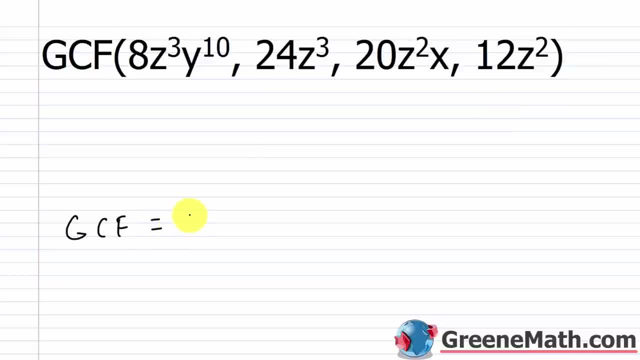 like that are going to speed up your work dramatically. So the number part is 4, and then for the variable parts, I have Z, Z, Z, and Z. Smallest exponent is a 2, right? Z cubed, Z cubed, Z squared, Z squared. 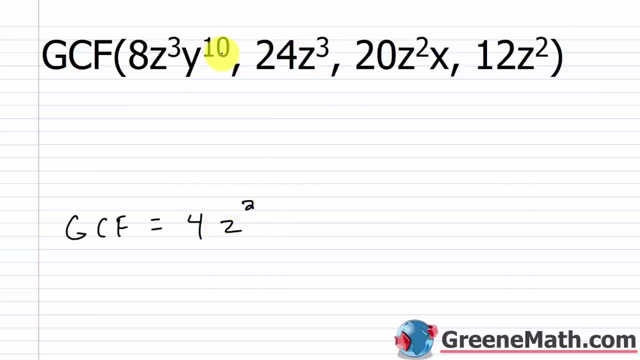 So Z squared, and then I have a Y to the 10th, no Y, I can stop. I have an X, no X anywhere else. 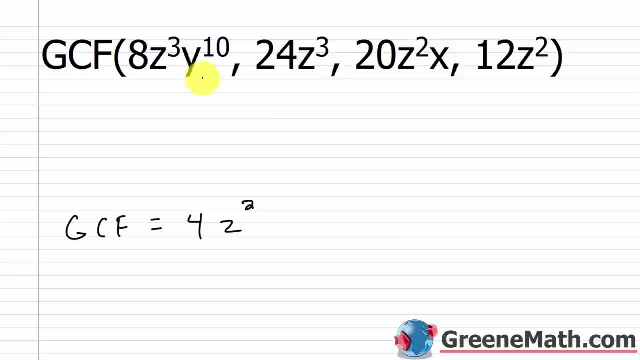 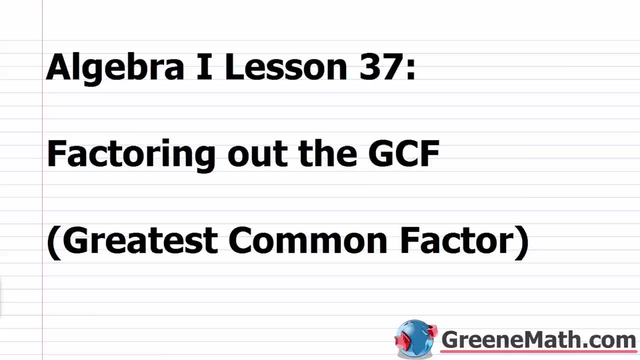 no y, I can stop. I have an x, no x anywhere else. so the GCF here is 4 z squared. Hello and welcome to Algebra 1, Lesson 37.. In this video we're going to learn about: 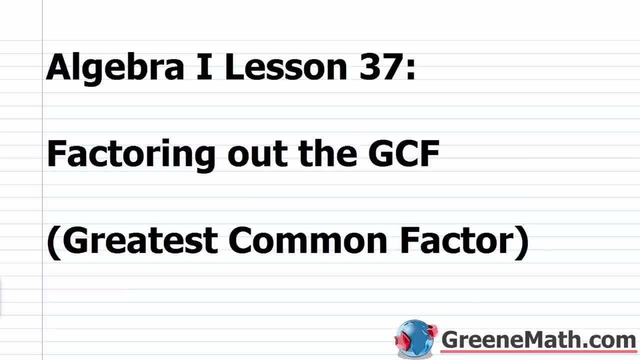 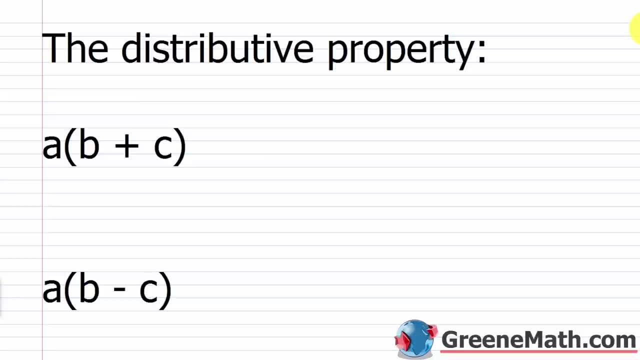 factoring out the GCF Again. this is known as the greatest common factor. So basically, in this lesson we're going to learn how to write a polynomial as a product. So this process is known to us as factoring, And essentially all 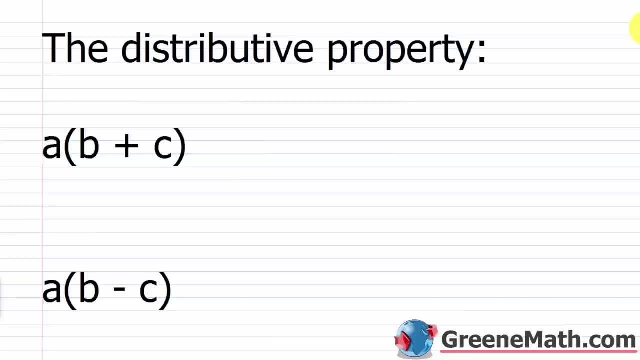 we're doing is we're reversing the distribution property. So let me kind of start off with a brief review of this, And at this point in Algebra 1, you should be very familiar with the distributive property. We use it all the time to simplify. 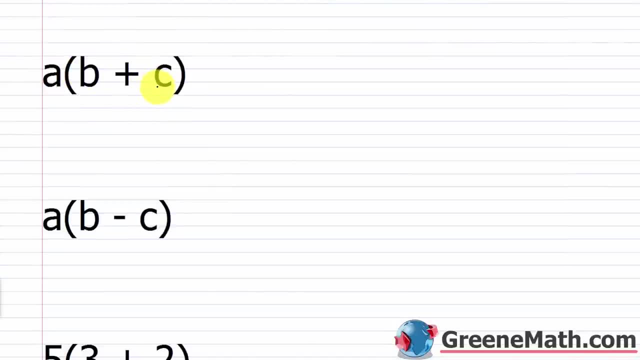 So if I have something like a times the quantity b plus c, we know that we can take a and multiply it by b, and I'd have ab, and then plus a times c, ac, And essentially all we're going to be doing is reversing. 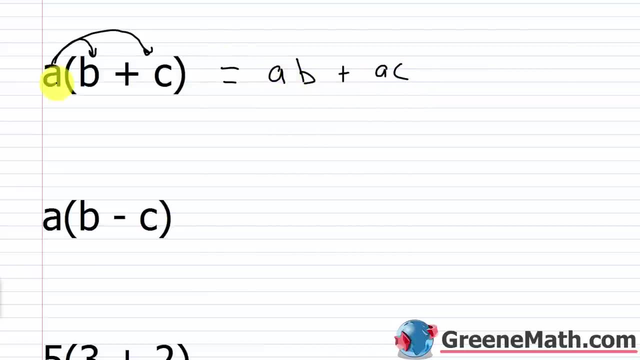 this. I'm going to see something that's ab plus ac and I'm going to go to a, outside of the parentheses, times that quantity b plus c, And we'll see how to do that in a minute. Another example: a times the quantity b minus c. 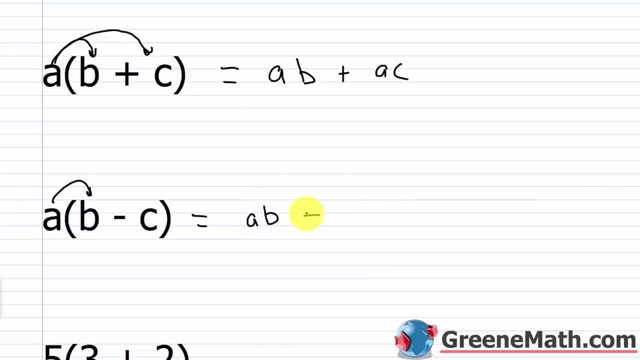 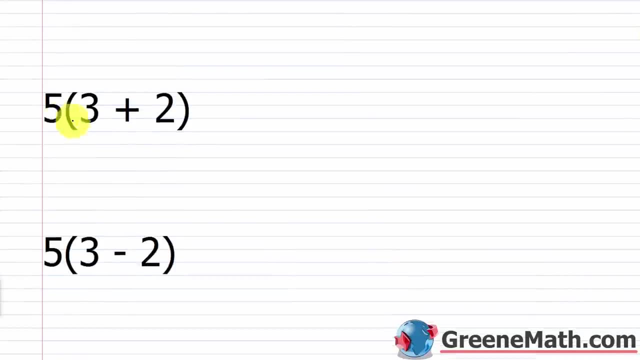 So we have a times b, this is ab minus a times c or ac. We can even do this with numbers involved. So we have 5 times the quantity 3 plus 2.. This is 5 times 3,, 5 times 3, plus. 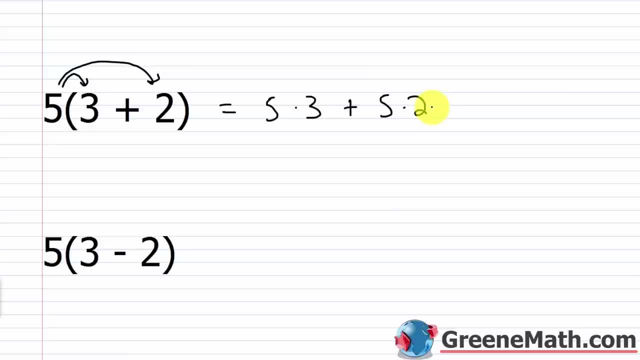 5 times 2.. When you get an example with numbers, it's easy to show that it's mathematically valid. If I do 3 plus 2 first, that's 5, 5 times 5 is 25.. 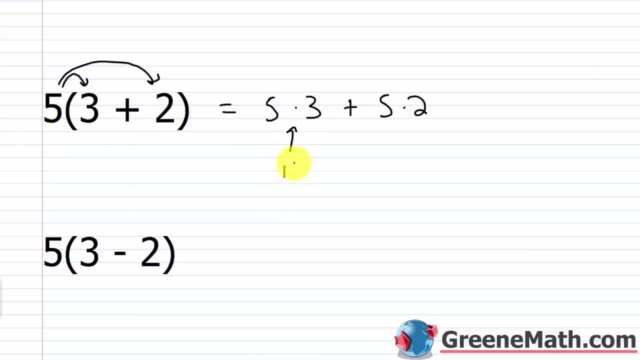 If I do it this way, 5 times 3 is 15, and then 5 times 2 is 10.. If I sum 15 and 10, I get 25 as well. So last one: here we have 5 times the quantity 3 minus 2,. 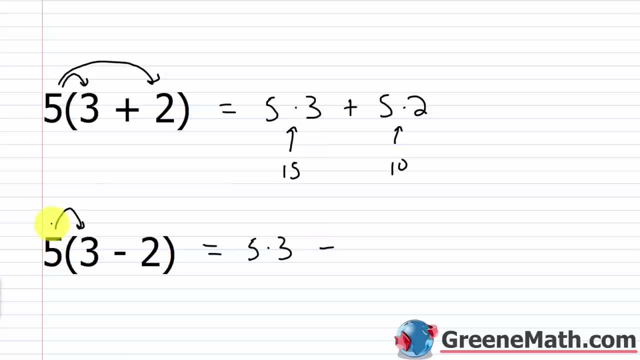 so 5 times 3,, 5 times 3 minus 5 times 2, and again, if you want to see that this is mathematically valid, 3 minus 2 is 1, 5 times 1 would be 5.. 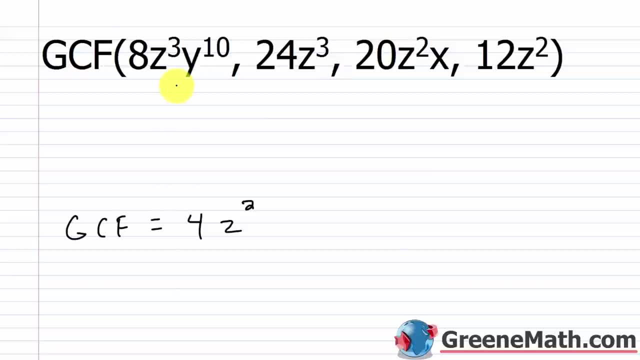 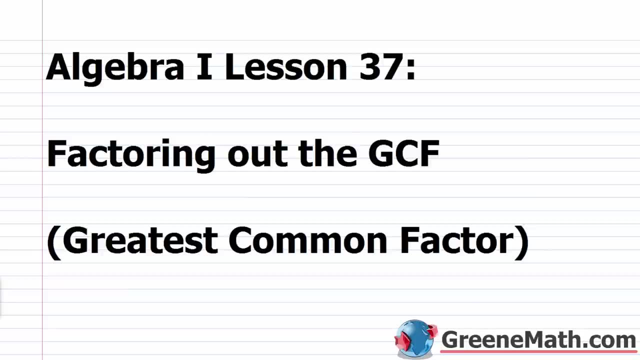 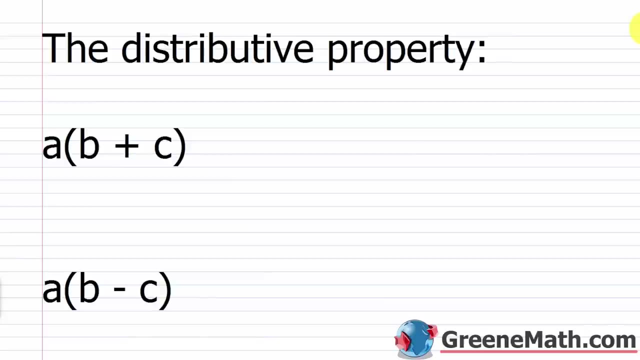 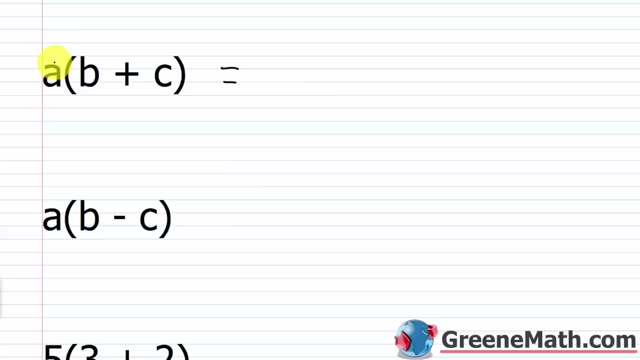 So the GCF here is 4Z squared. Hello, and welcome to Algebra 1, Lesson 37. In this video, we're going to learn about factoring out the GCF. Again, this is known as the greatest common factor. So basically in this lesson, we're going to learn how to write a polynomial as a product. This process is known to us as factoring. And essentially, all we're doing is we're reversing the distributive property. So let me kind of start off with a brief review of this. And at this point in Algebra 1, you should be very familiar with the distributive property. We use it all the time to simplify. So if I have something like A times the quantity B plus C, we know that we can take A and multiply it by B, and I'd have AB, and then plus A times C. 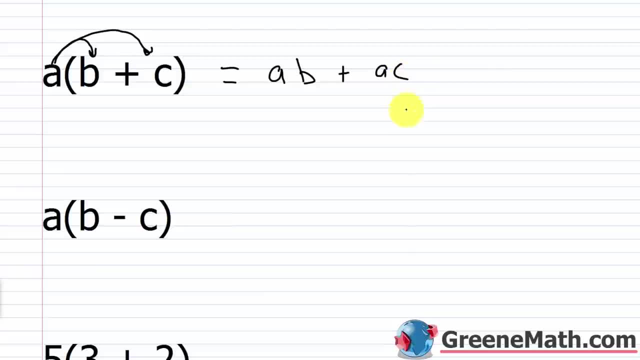 AC. And essentially, all we're going to be doing is reversing this. I'm going to see something that's AB plus AC, and I'm going to go to A outside of the parentheses times that quantity B plus C. And we'll see how to do that in a minute. Another example, A times the quantity 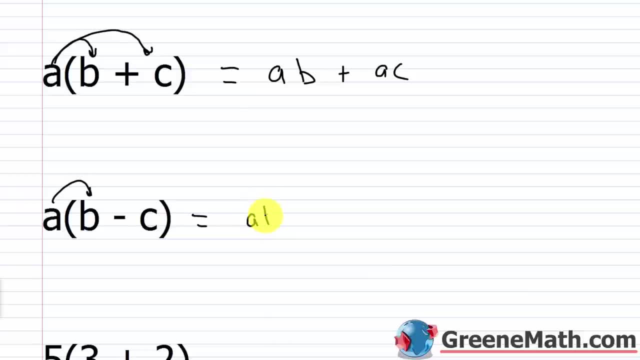 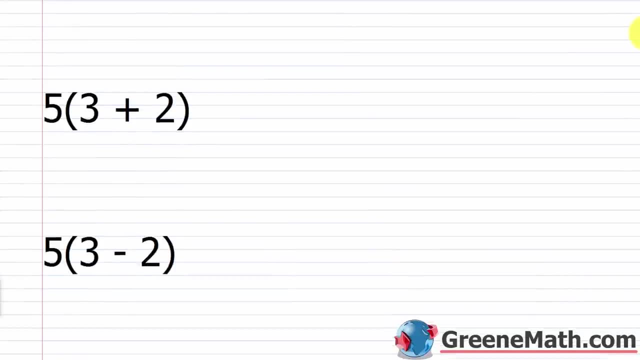 B minus C. So we have A times B, this is AB, minus A times C, or AC. We can even do this with numbers involved. So we have 5 times the quantity 3 plus 2. 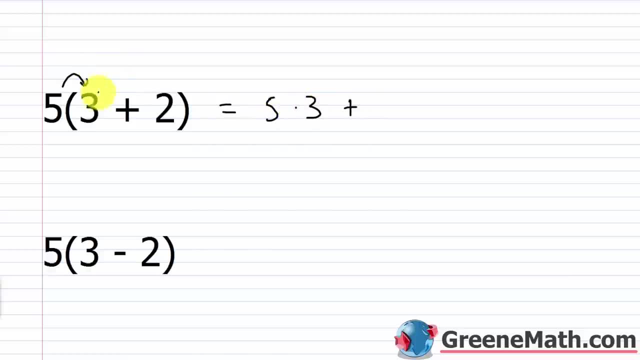 This is 5 times 3, 5 times 3, plus 5 times 2. 5 times 2. When you get an example with numbers, it's easy to show that it's mathematically valid. If I do 3 plus 2 first, that's 5, 5 times 5 is 25. If I do it this way, 5 times 3 is 15, and then 5 times 2 is 10. If I sum 15 and 10, I get 25 as well. So last one here, we have 5 times the quantity 3 minus 2. 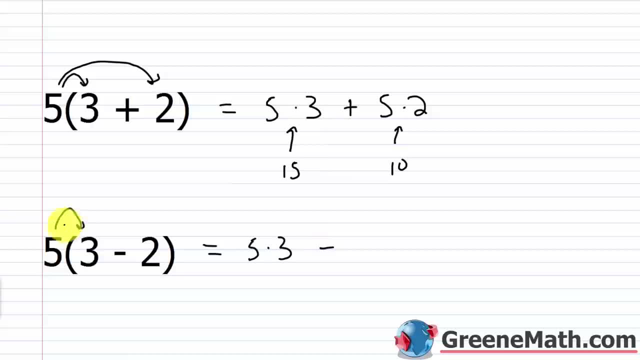 So 5 times 3 plus 5 is 15. And then 5 times 3 is 15. And then 5 times 2 is 15. And then 5 times 5 times 3, 5 times 3, minus 5 times 2, 5 times 2. 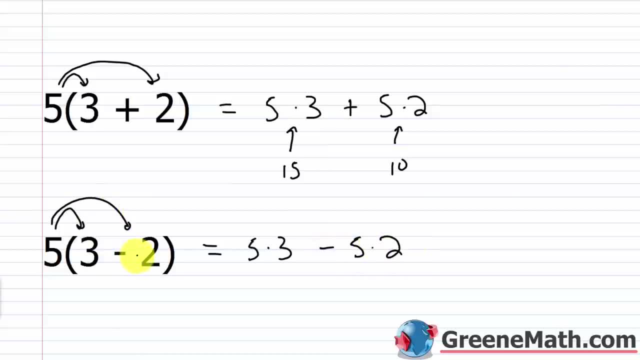 And again, if you want to see that this is mathematically valid, 3 minus 2 is 1, 5 times 1 would be 5. If I look here, 5 times 3 is 15. 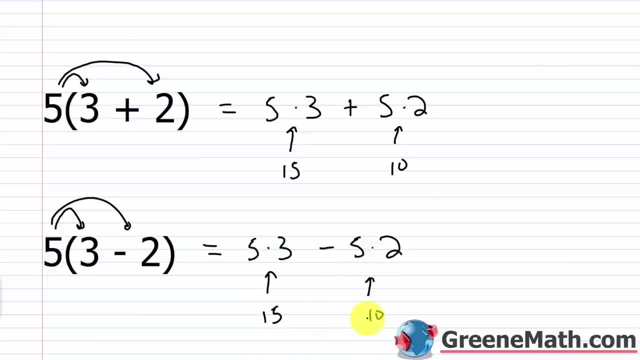 Again, 5 times 2 is 10. 15 minus 10 is again 5. 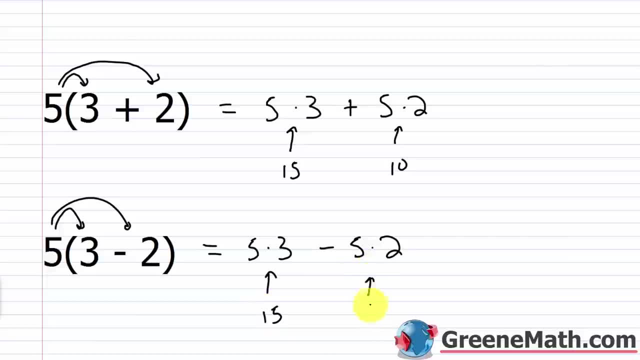 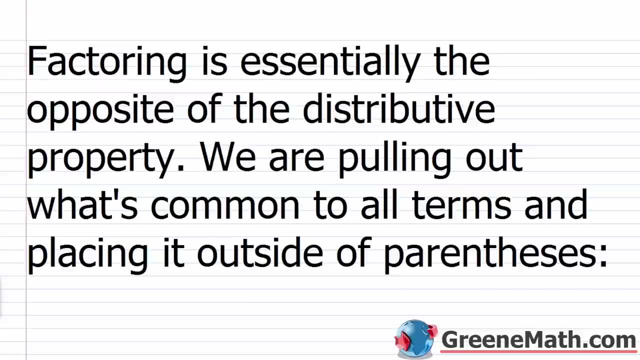 If I look here, 5 times 3 is 15, again 5 times 2 is 10,. 15 minus 10 is again 5.. Alright, so factoring is essentially the opposite of the distributive property. So we are. 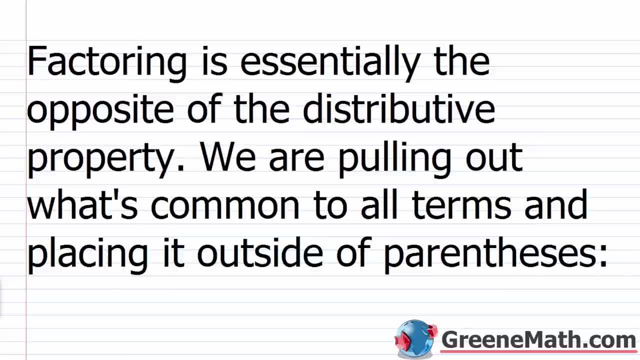 pulling out what's common to all terms and placing it outside of parentheses. This is something you're going to do for the rest of your life. It's not something that you're just going to do for one little section in Algebra 1, and then you can kind of 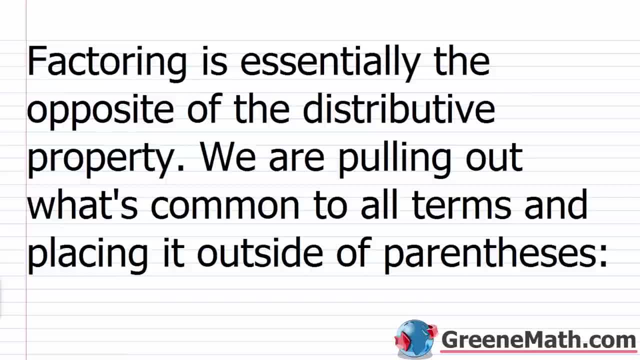 forget about it. You will become very, very good at factoring and kind of. as you move forward, the factoring gets tougher and tougher. The stuff we're going to look at in this lesson is going to be very, very simple. 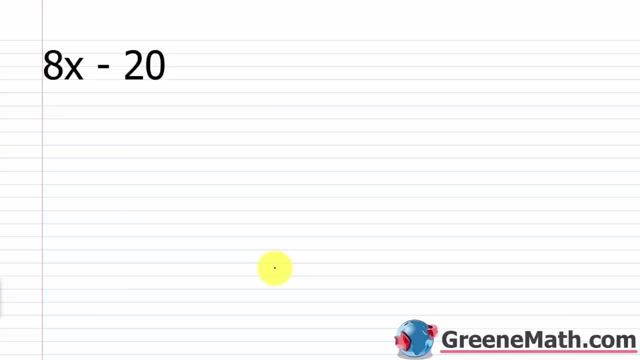 very, very straightforward, Alright. so let's take a look at our first example and again, what we want to do here is factor out the GCF, the greatest common factor. So if we're going to factor out the greatest common factor, 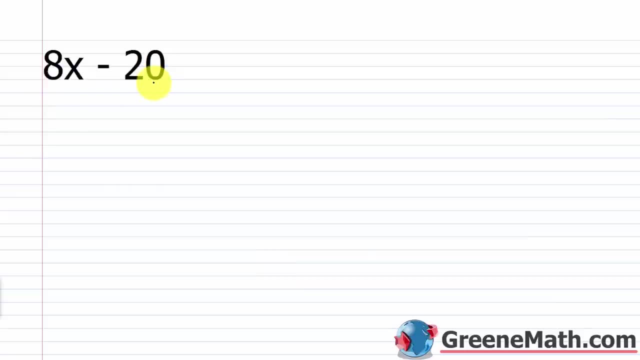 the first thing we need to do is find the greatest common factor. So what is that here? So the GCF is equal to what? Well, if I look at this first term here, I have 8x. And if I look at the second term, I have 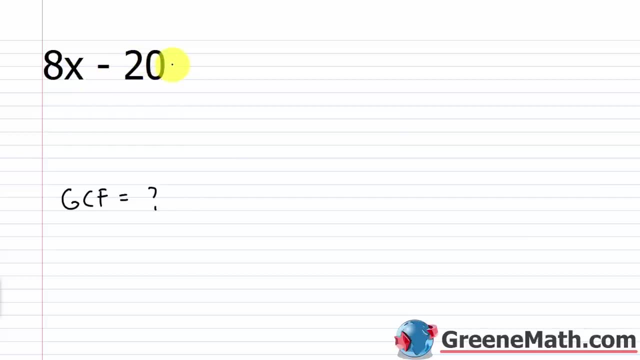 20. Now there's no x involved in both terms, so it's not going to be part of the greatest common factor. So now I'm just thinking about 8, and I'm thinking about 20.. So 8, I can think of as what? 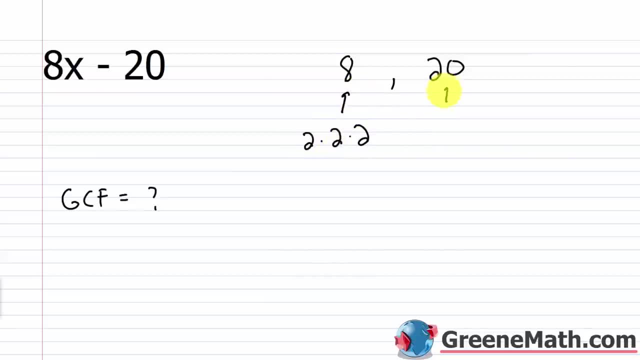 It's 2 times 2 times 2, and 20 is what It's 2 times 2 times 5.. So it's pretty easy to see that the greatest common factor here is 4, right- 2 times 2.. 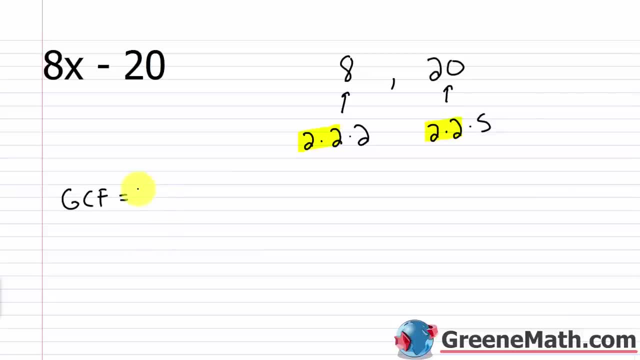 Alright. so once we know that, we kind of move on to our next step, Before I kind of get into that, let me one more time show you the distributive property with something we've already seen. So let's say I have again a times. 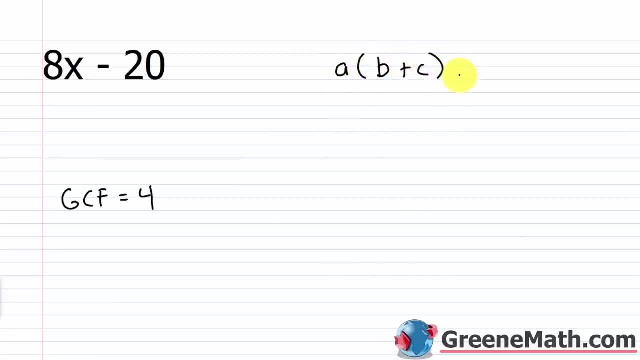 the quantity b plus c. So I take a, I multiply it by b, I get ab. I take a, I multiply it by c, I get plus ac. Now what if I was to start out with ab plus ac And I want to go into this format? 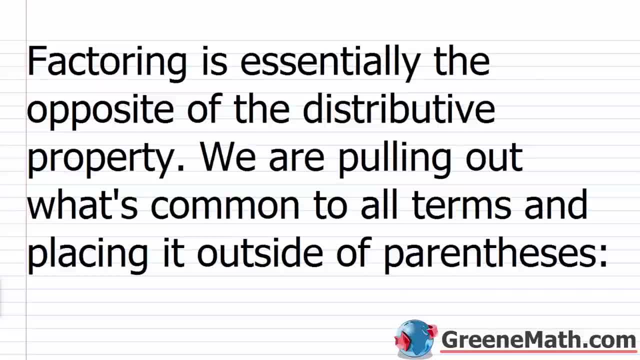 All right, so factoring is essentially the opposite of the distributive property. So we are pulling out what's common to all terms and placing it outside of parentheses. 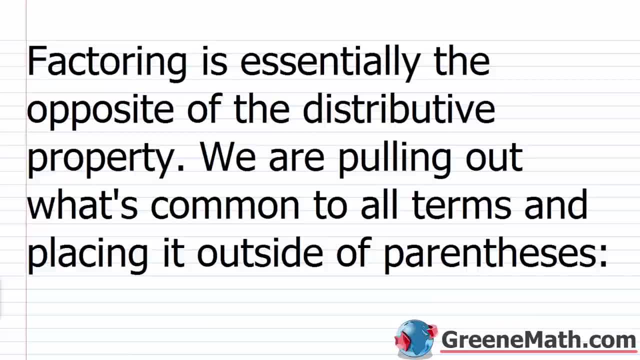 This is something you're going to do for the rest of your life. It's not something that you're just going to do for, you know, 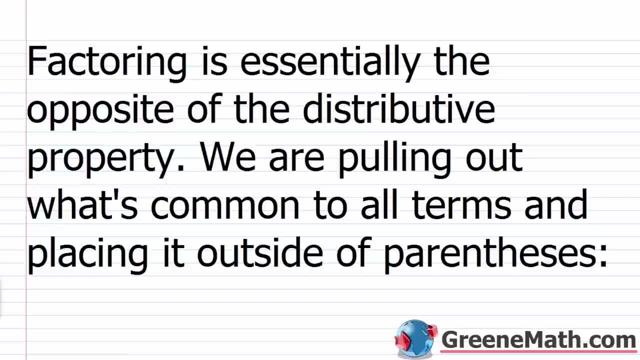 You will become very, very good at factoring. And kind of as you move forward, the factoring gets tougher and tougher. 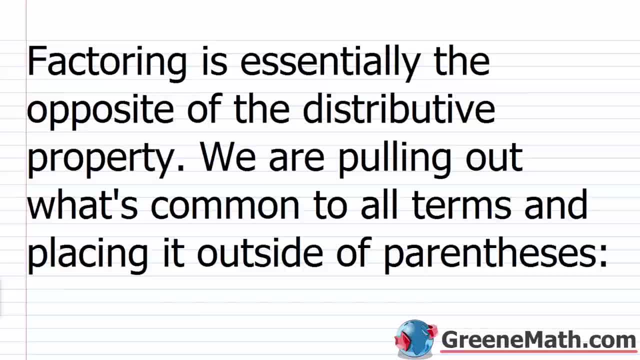 The stuff we're going to look at in this lesson is going to be very, very simple, very, very straightforward. 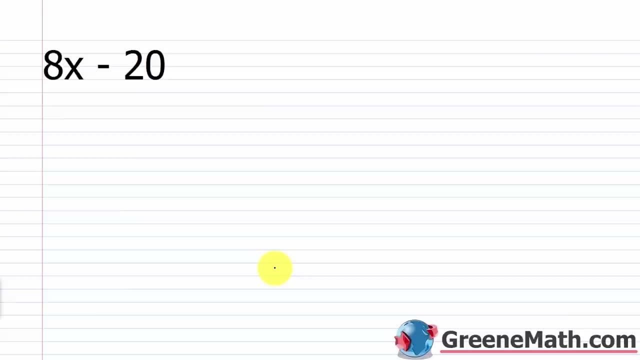 All right, so let's take a look at our first example. And again, what we want to do here is factor out the GCF, the greatest common factor. So if we're going to do this, if we're going to factor out the greatest common factor, the first thing we need to do is find the greatest common factor. So what is that here? So the GCF is equal to what? 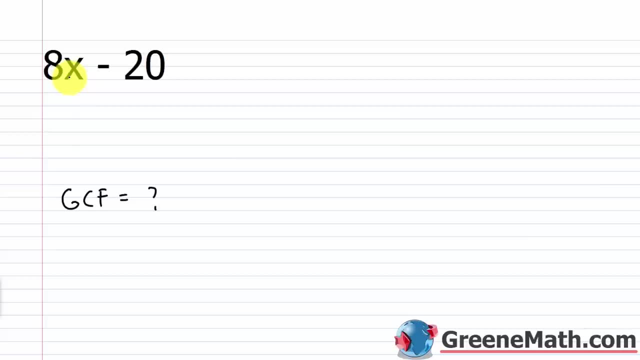 Well, if I look at this first term here, I have 8x. And if I look at the second term, I have 20. 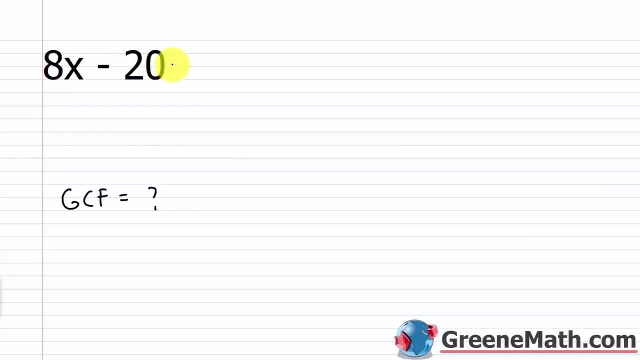 Now, there's no x involved in both terms, so it's not going to be part of the greatest common factor. 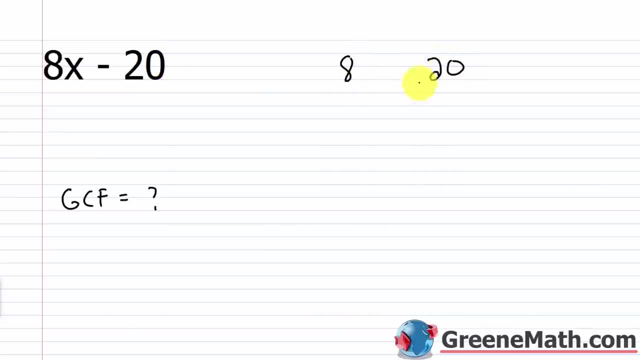 So now I'm just thinking about 8 and I'm thinking about 20. So 8 I can think of as what? It's 2 times 2 times 2, and 20 is what? It's 2 times 2 times 5. 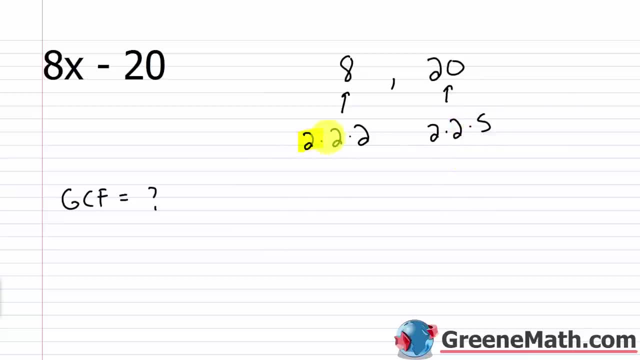 So it's pretty easy to see that the greatest common factor here is 4, right? 2 times 2. 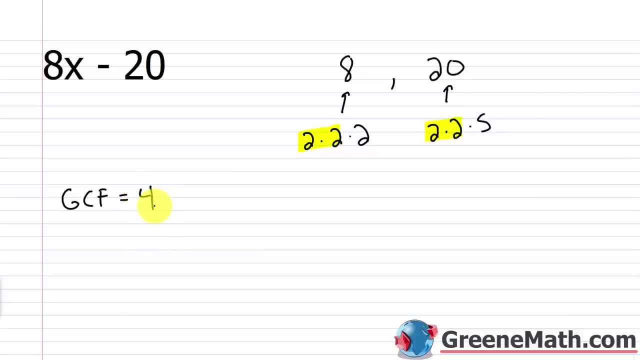 All right, so once we know that, we kind of move on to our next step. And before I kind of get into that, let me one more time show you the distributive property with something we've already seen. 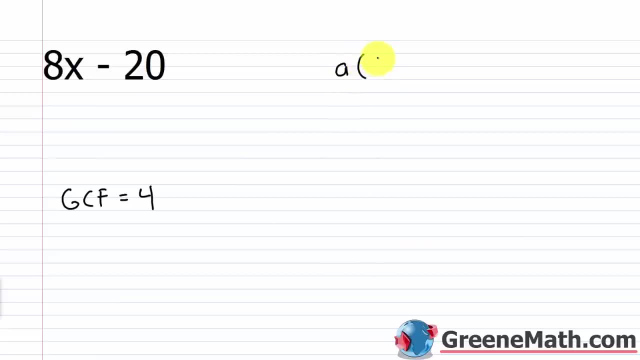 So let's say I have, again, a times the quantity, b plus c. 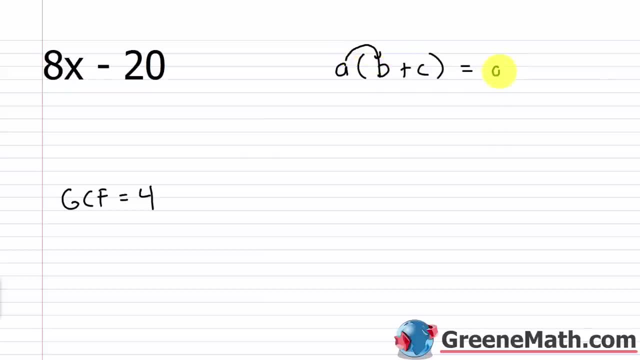 So I take a, I multiply it by b, I get ab. I take a, I multiply it by c, I get plus ac. 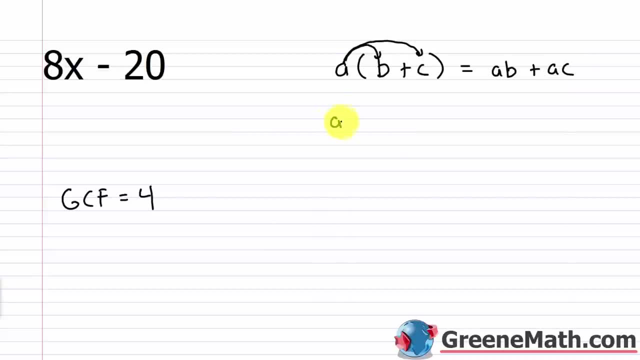 Now, what if I was to start out with ab plus ac? And I want to go into this format. 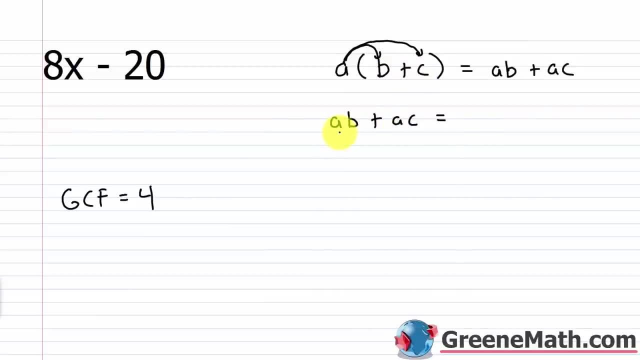 In other words, I want what's common, or the greatest common factor, which in this case is a, to be outside of a set of parentheses. 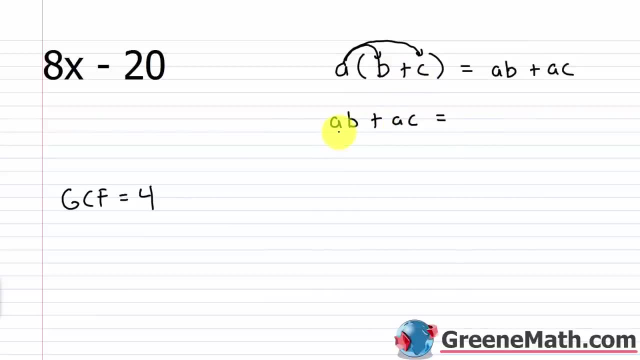 In other words, I want what's common, or the greatest common factor, which in this case is a, to be outside of a set of parentheses. How do I get this space and this space? What do I do? Well, there's kind of. 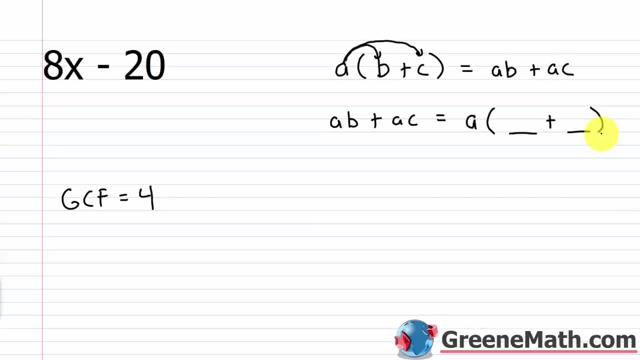 two ways you can think about it. The easiest way to do it would be just to take each term here and divide by what you're putting outside of the parentheses. In other words, if I took ab and I divided by a, I get b. If I took ac. 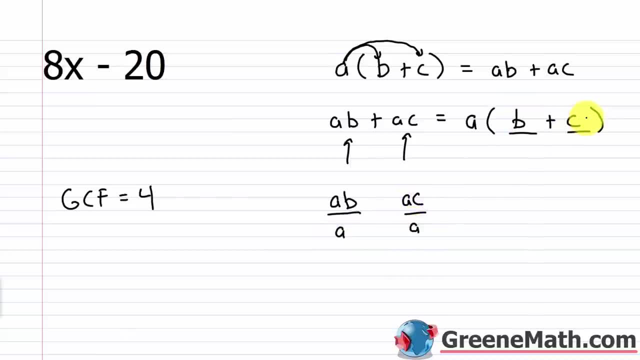 and I divided by a, I would get c. And the reason that works is because, remember, division is the opposite of multiplication. So if I take ab and I divide by a, I get b. If I was to multiply a by b, I get ab. 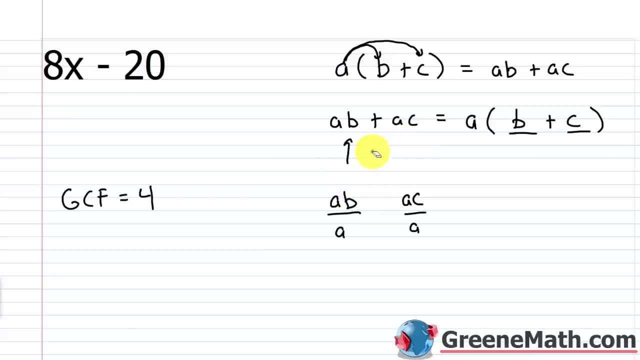 right back. It's just the opposite of multiplication. So the other thing that you can do, if you don't like doing it that way, you could take this ab plus ac and you could just think about: okay, I'm taking this a. 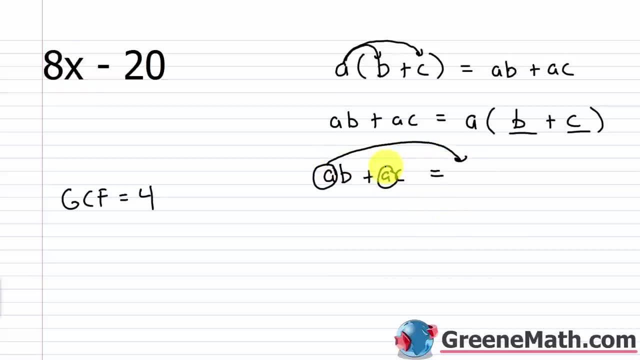 that's common to both, and I'm placing it outside of a set of parentheses. So that's going to go there. Then I could say: well, what's left after I take that a out? Well, there's just a b there, and then there's just a c there. 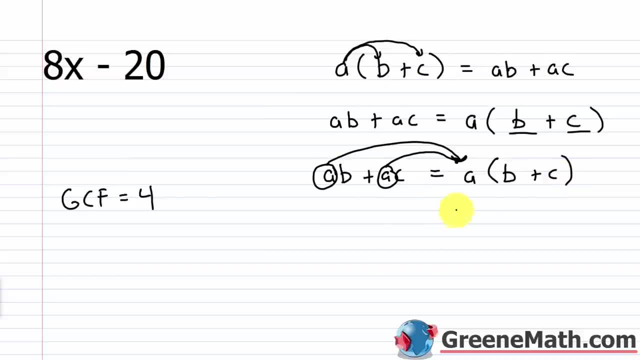 That works just as well. Taking this example and applying it to this, what are we going to see? Well, if I have 8x minus 20 and I know my GCF is 4, so let's write 4 out there. Well, again, I can. 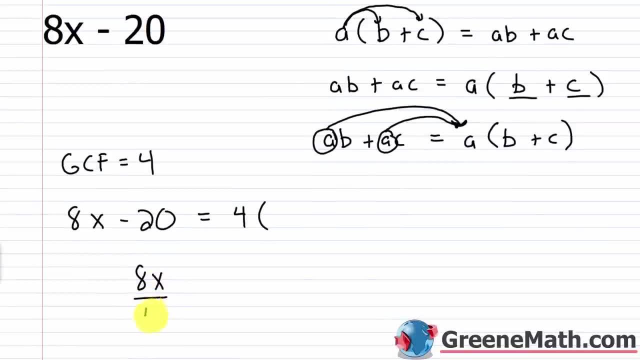 start out by just saying: okay, each term divided by the GCF, 8x over 4, is 2x, and then minus we'd have 20 over 4.. That's going to be 5.. So I've just factored my first polynomial. 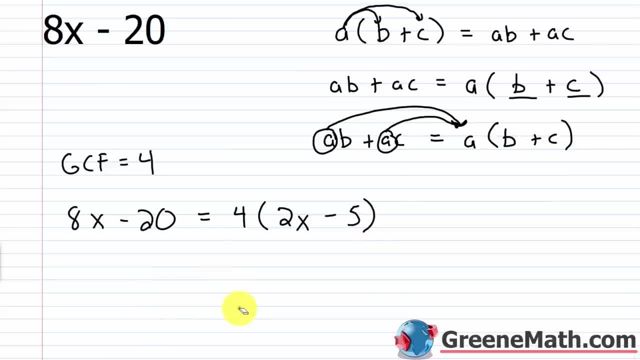 I took 8x minus 20 and I said: this is equal to 4 times the quantity 2x minus 5.. And again, if you want to check this, it's very, very easy. All you have to do is do the multiplication. 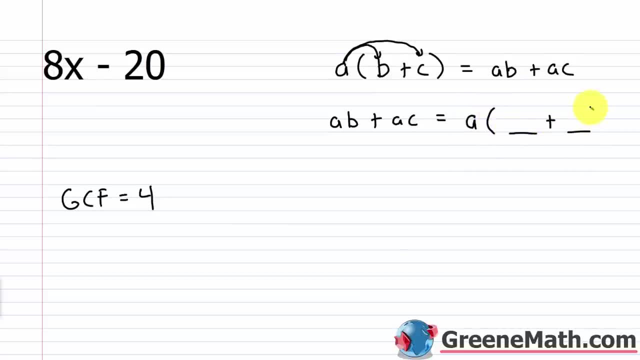 How do I get this space? And this space? What do I do? Well, there's kind of two ways you can think about it. 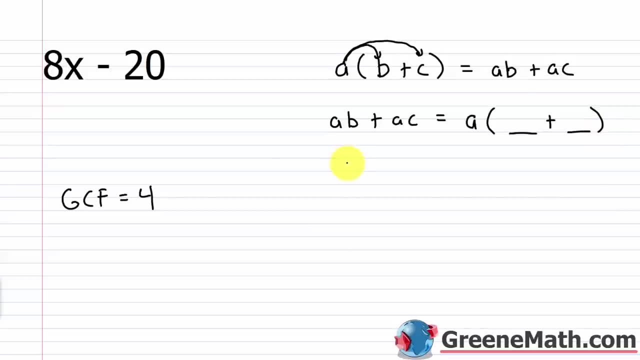 The easiest way to do it would be just to take each term here and divide by what you're putting outside of the parentheses. 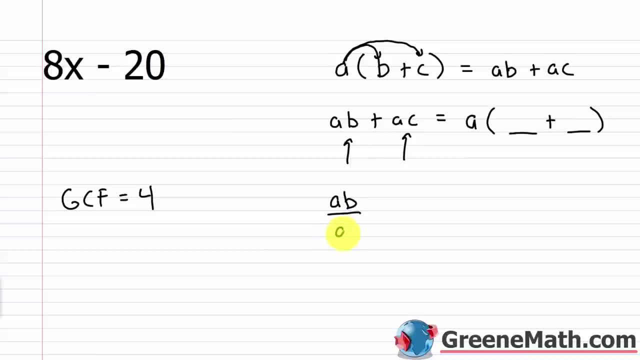 In other words, if I took ab and I divided by a, I get b. 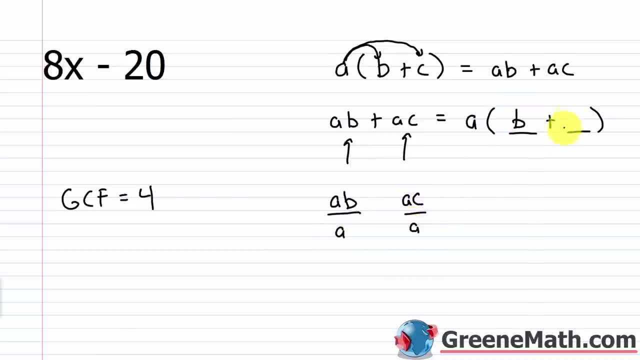 If I took ac and I divided by a, I would get c. 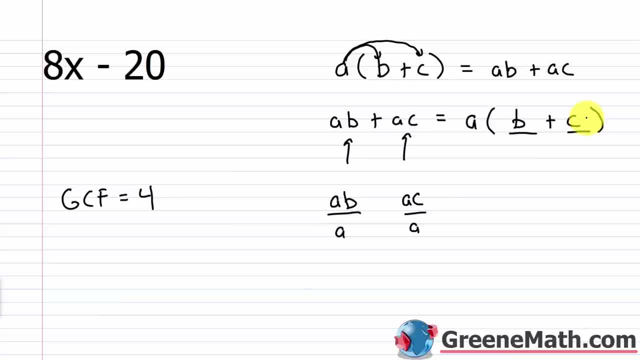 And the reason that works is because, remember, division is the opposite of multiplication. 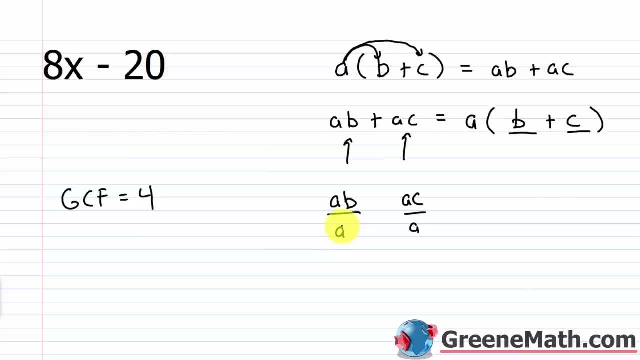 So if I take ab, and I divide by a, I get b. If I was to multiply a by b, I get ab right back. 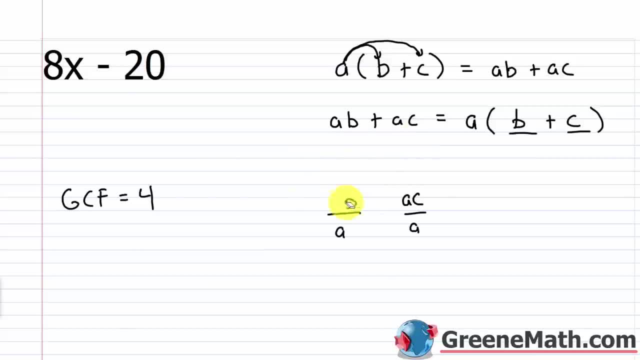 It's just the opposite operation. So the other thing that you can do, if you don't like doing it that way, you could take this, ab plus ac, and you could just think about, okay, I'm taking this a, that's common to both, and I'm placing it outside of a set of parentheses. So that's going to go there. Then I could say, well, what's left after I, take that a out? Well, there's just a b there, and then there's just a c there, right? That works just as well. 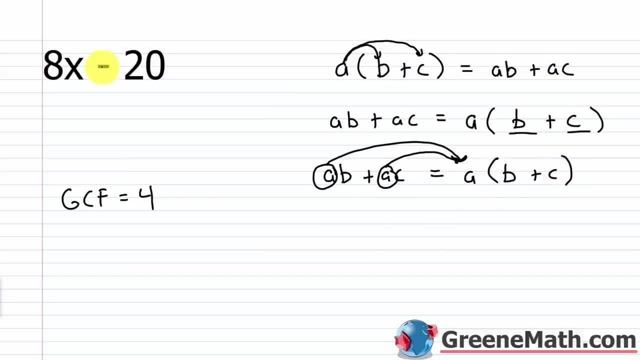 So now taking this example and applying it to this, what are we going to see? 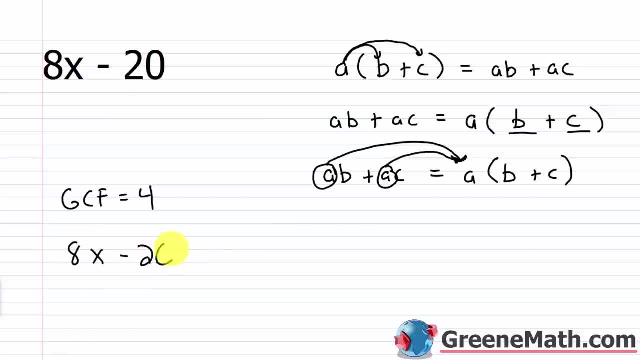 Well, if I have 8x minus 20, and I know my GCF is four, so let's write four out there. Well, again, I can start out by just saying, 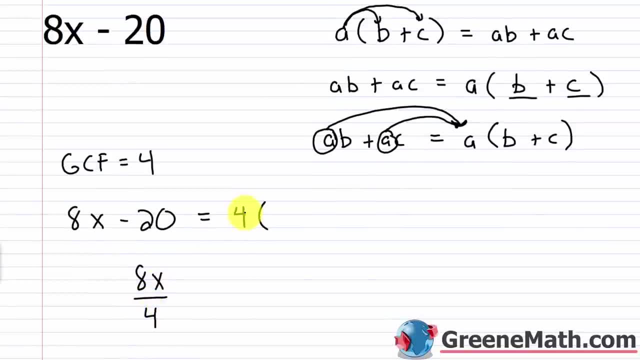 each term divided by the GCF. 8x over four is 2x. And then, minus, we'd have 20 over four. That's going to be five. 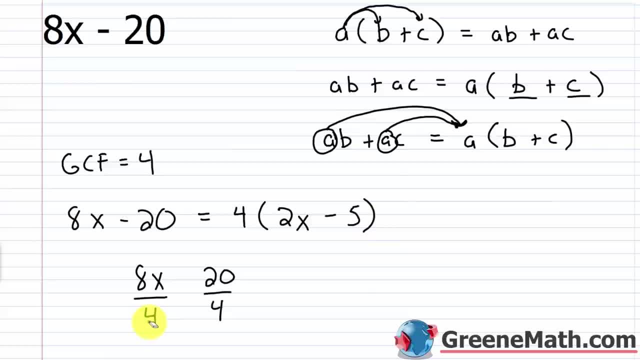 So I've just factored my first polynomial. I took 8x minus 20, and I said this is equal to four times the quantity 2x minus five. 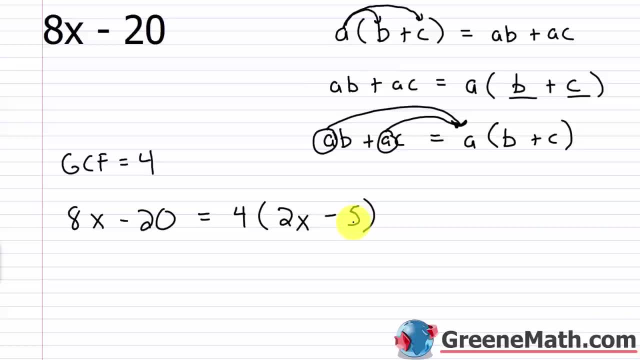 And again, if you want to check this, it's very, very easy. 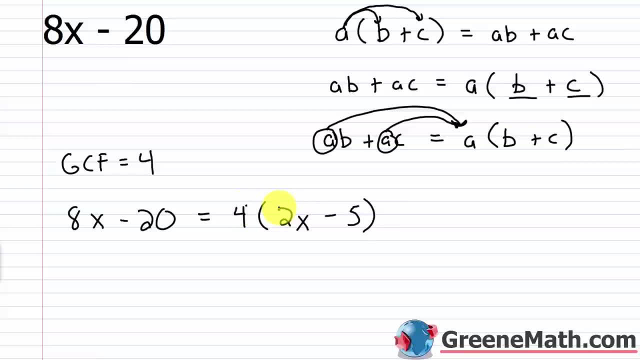 All you have to do is do the multiplication. Okay, so four times 2x is 8x. 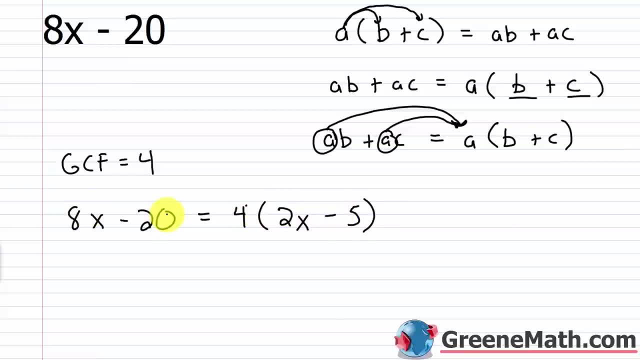 Okay, so 4 times 2x is 8x. 4 times negative, 5 is negative 20.. So bam, right, there, I know I got the right answer. Now one thing I want to draw your attention to. A lot of students will. 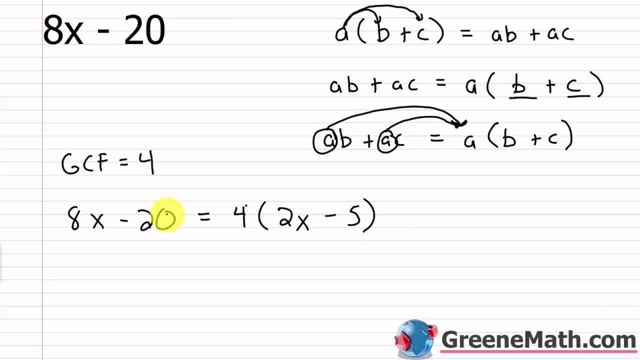 understand how to factor, but they'll make a mistake and not get the correct GCF. So, for example, let's say I put 8x minus 20 and I only factored out a 2. So I put a 2 here. 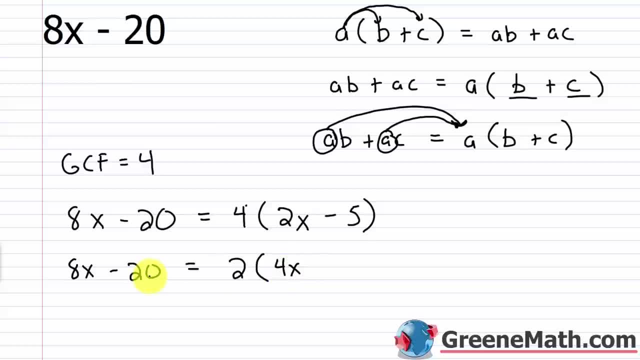 So then, 8x divided by 2 is 4x. 20 divided by 2 is 10.. So minus 10.. If your teacher asks you to factor out the GCF, this is not the right answer. This is wrong Because I only factored. 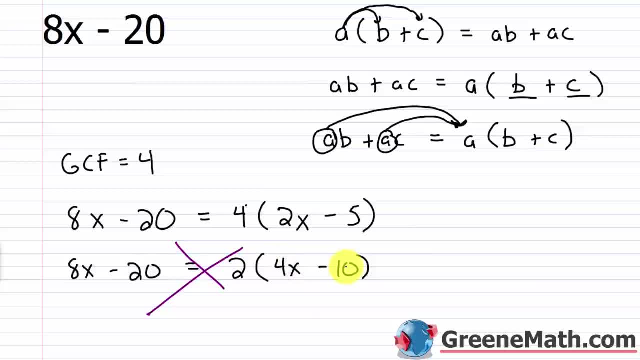 out a 2. I have 2- that's common to each term inside the parentheses that can come out, So you might end up getting the wrong answer even though you factor correctly, because you didn't pull everything out that you could. So pay close attention to that. 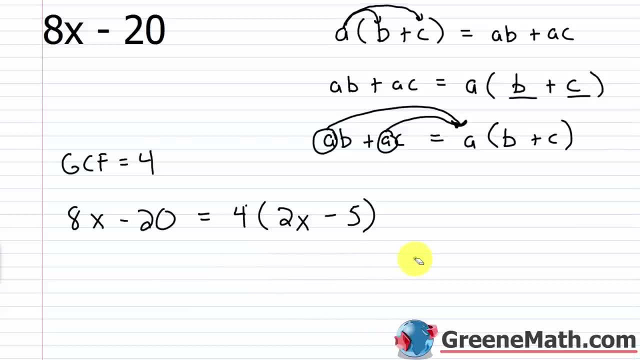 Now the other thing I want to do. I just want to show you really quickly the other method that I kind of used over here, So I could have written this as 4 times 2x minus 4 times 5.. And again this makes: 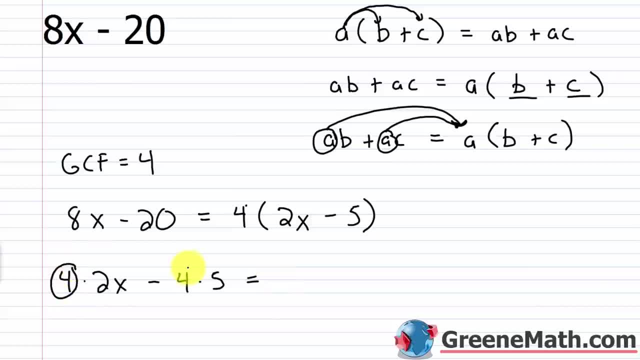 it easier to visualize, I'm pulling out a 4. And again that's going outside of a set of parentheses. So that's going to go there, And then what's left? Here it would be 2x And then minus here. 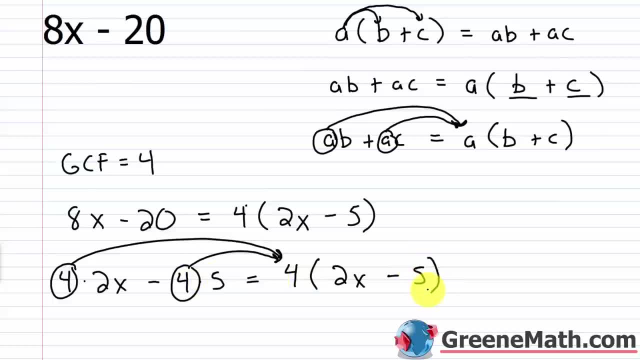 it would be 5.. So, again, I get the same thing either way. So, however you want to look at that, those are the two basic methods you can use to take that polynomial and write it in factored form. Alright, let's take a look at another one. 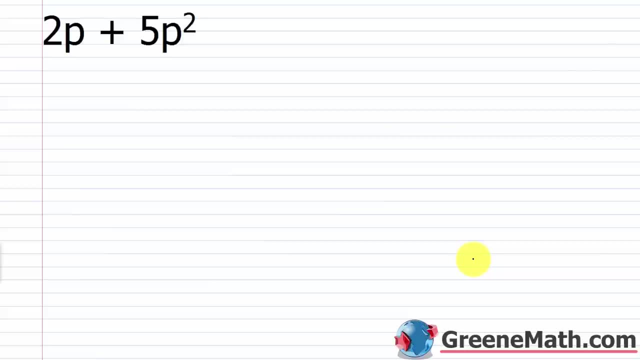 So we have 2p plus 5p squared. So again, the first question is: what is the greatest common factor? And it's pretty easy here, because 2 is a prime number and 5 is a prime number. So the only thing these have in common, number-wise. Four times negative five is negative 20. So bam, right there, I know I got the right answer. 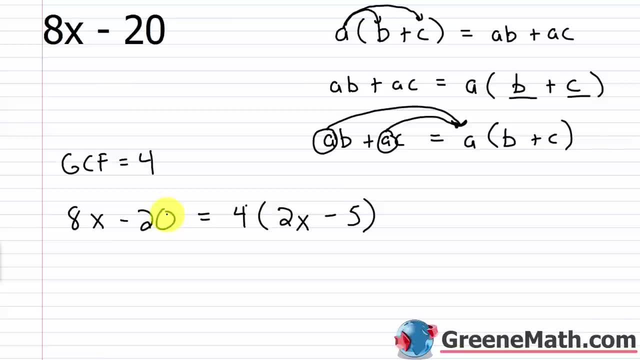 Now, one thing I want to make sure you know about this, and this is one thing I want to draw your attention to. A lot of students will understand how to factor, 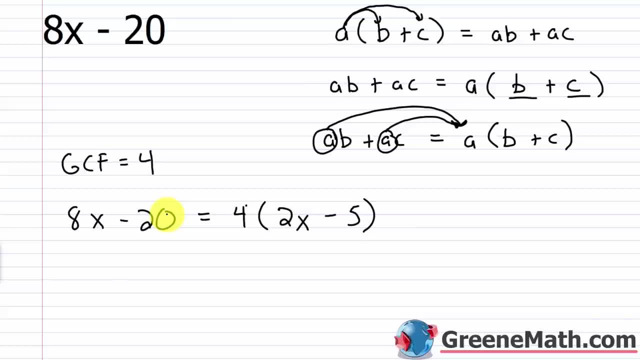 but they'll make a mistake and not get the correct GCF. 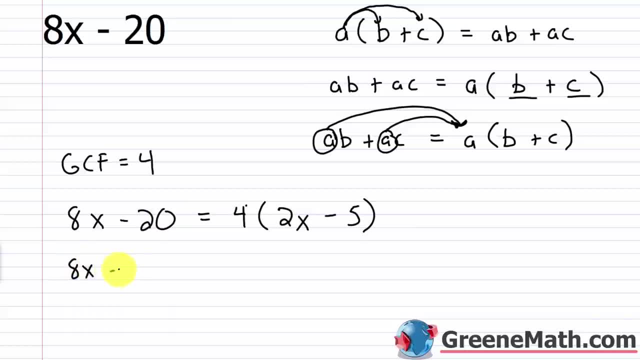 So for example, let's say I put 8x minus 20, and I only factored out a two. So I put a two here. 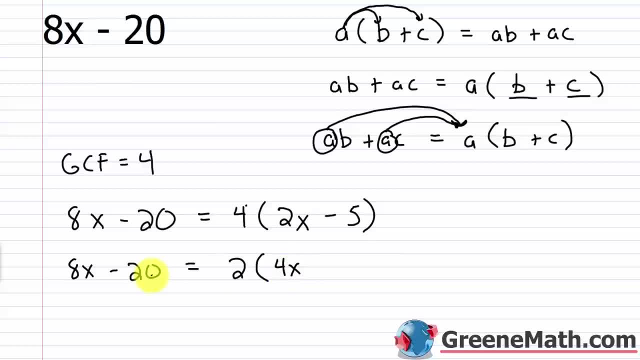 So then 8x divided by two is 4x. 20 divided by two is 10, so minus 10. 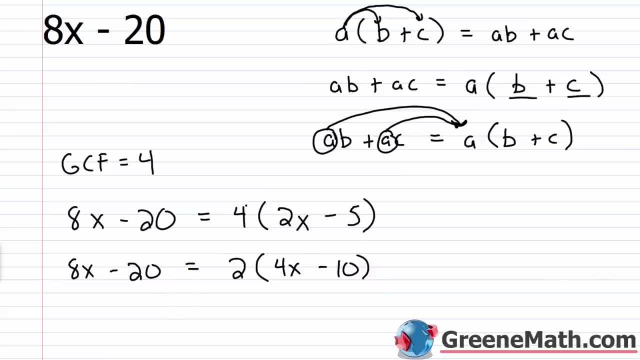 If your teacher asks you to factor out the GCF, this is not the right answer. This is wrong. Because I only factored out a two. 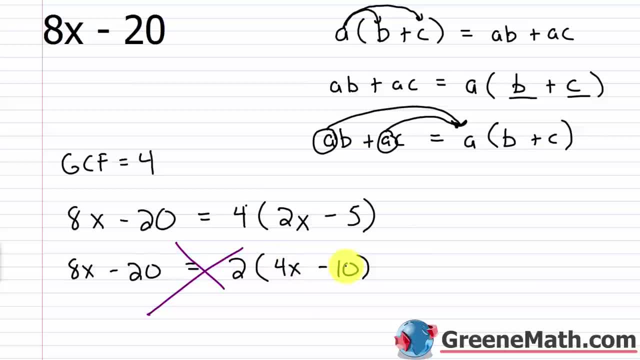 I have two that's common to each term inside the parentheses that can come out. 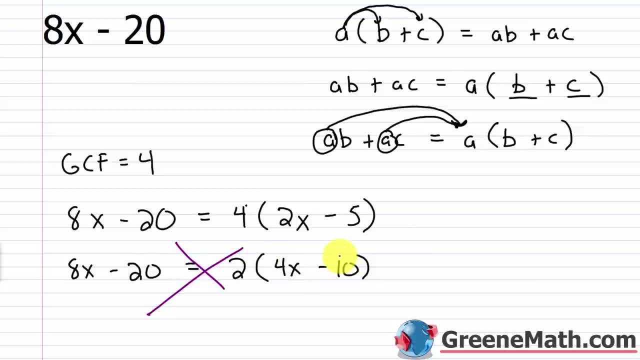 So you might end up getting the wrong answer, even though you factor correctly, because you didn't pull everything out that you could. 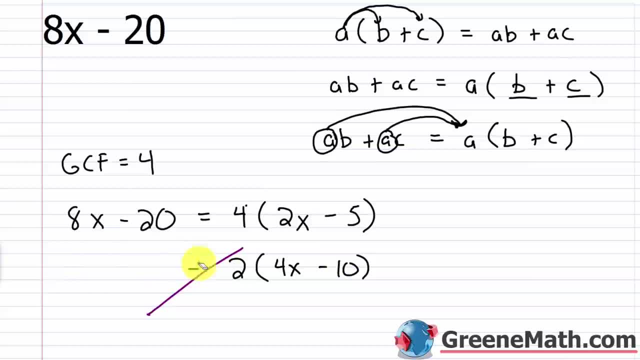 So pay close attention to that. Now, the other thing I want to do, 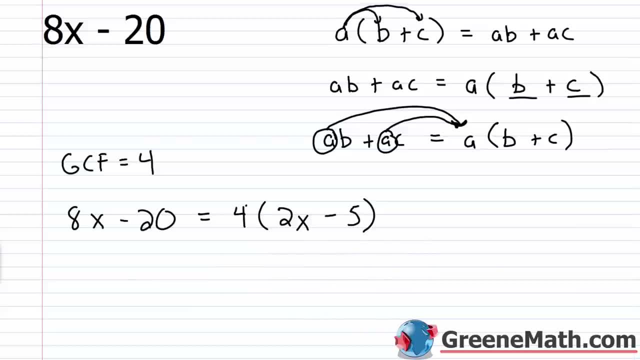 I just want to show you really quickly the other method that I kind of used over here. 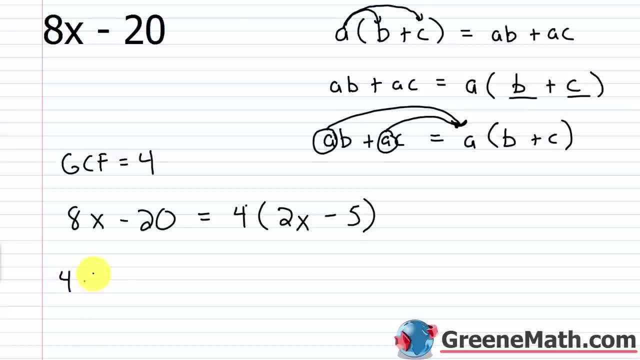 So I could have written this as four times 2x minus four times five. 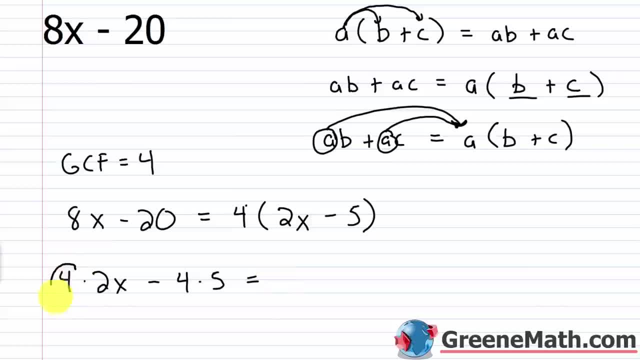 And again, this makes it easier to visualize. I'm pulling out a four. And again, that's going outside of a set of parentheses. 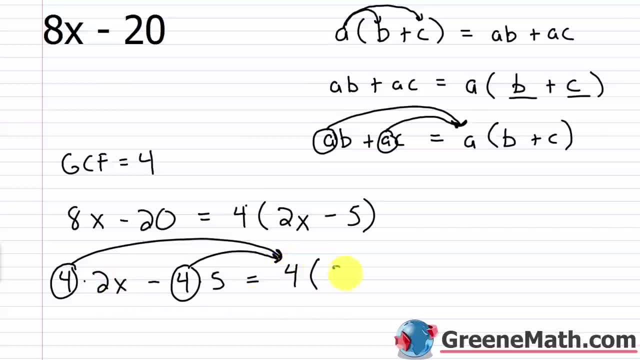 So that's going to go there. And then what's left here will be 2x. And then minus here, it would be five. So again, I get the same thing either way. So however you want to look at that, those are the two basic methods you can use 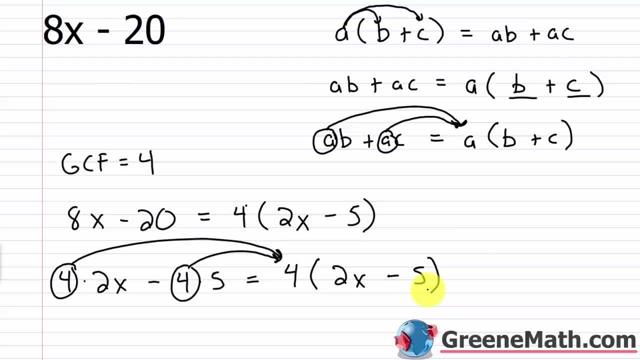 to take that polynomial and write it in factored form. All right, let's take a look at another one. So we have 2p plus 5p squared. 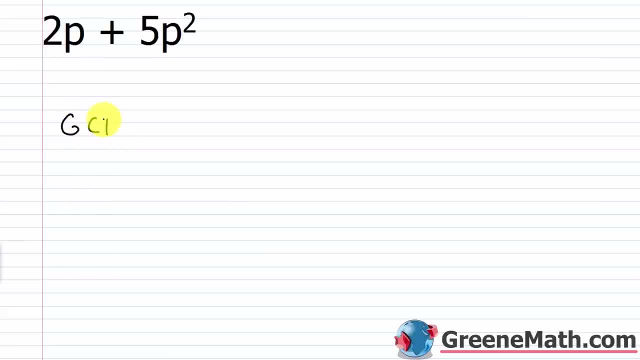 So again, the first question is, what is the greatest common factor? And it's pretty easy here because two is a prime number and five is a prime number. 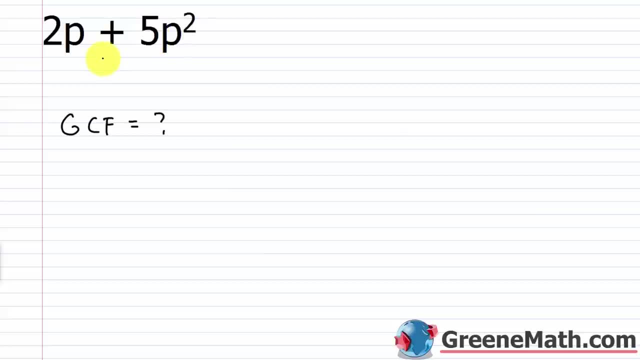 So the only thing these have in common number-wise would just be the number one. 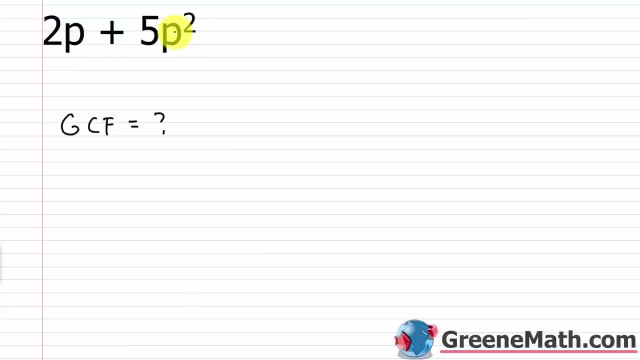 So kind of moving on, we see that they each have the variable p. One is p to the first power, one is p squared. 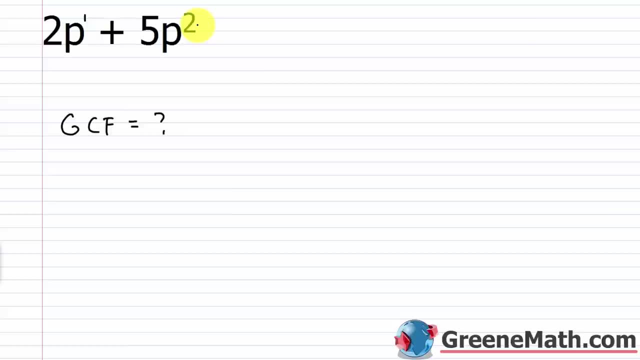 So you use the exponent on the variable that's smallest. In this case, that's going to be one. So the greatest common factor is p. So the greatest common factor is p. So the greatest common factor is just p. 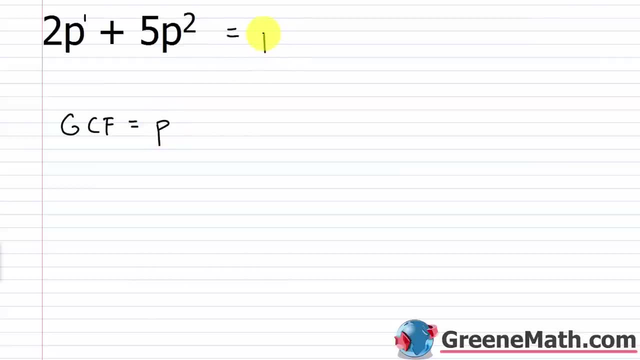 All right, so to factor this guy out, again, I'm going to put p outside of a set of parentheses. So inside, what am I going to use to fill these two spaces? Again, I can do it two ways. 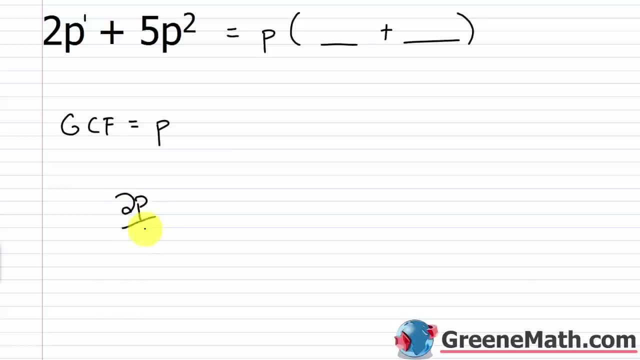 I can divide 2p by p. 2p by p, that's going to give me 2. 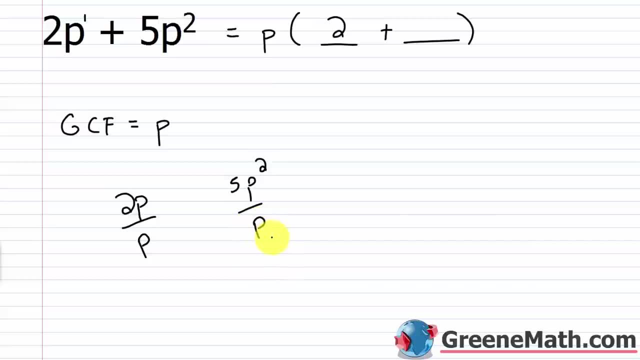 And then I can divide 5p squared by p. That's going to give me, this will cancel with this, 5p, so 5p. 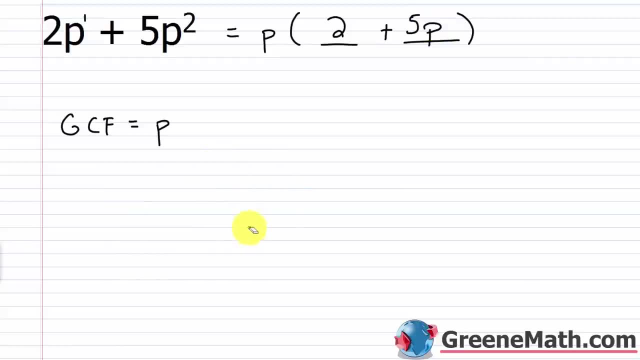 And then the other way, again, if you're more comfortable doing it this way, you could also say, okay, well, I have 2 times p. I'm going to write this in a different color. And then plus, I have 5 times p times p. 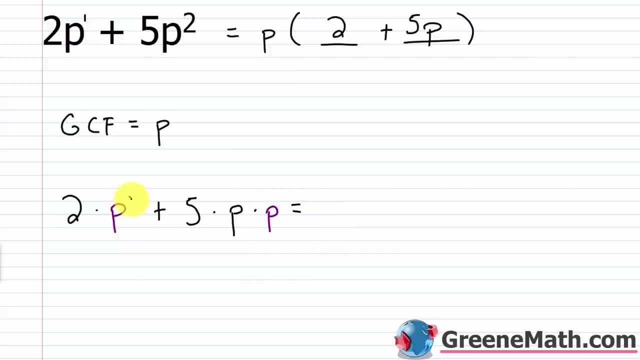 So then it makes it completely obvious that I'm going to pull this out in each case, pull this out, place it outside of the parentheses, and then what's left? 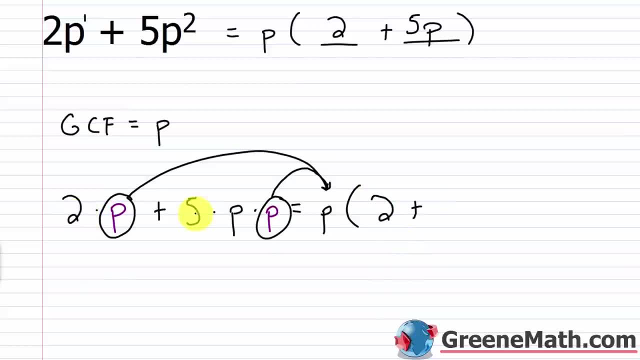 So I'd have a 2 here, plus, and here I'd have 5p. So either way you want to do it, you would get p times the quantity 2 plus 5p. 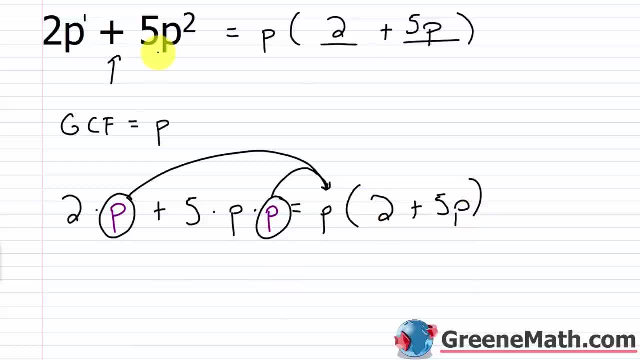 And if it makes you feel more comfortable, because I know none of this is in standard form, you could flip the order of this to begin. 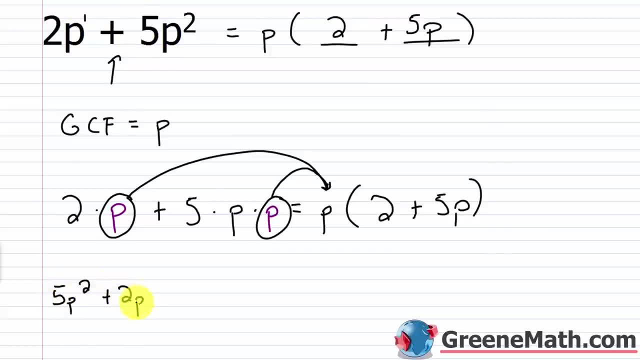 So you could say 5p squared plus 2p is equal to, and then you'd have p times, flip the order of this, 5p plus 2. And again, you can check it with multiplication. p times 5p is 5p. 5p squared. p times 2 is 2p. So you get 5p squared plus 2p. All right, so here's another thing that trips students up a lot. 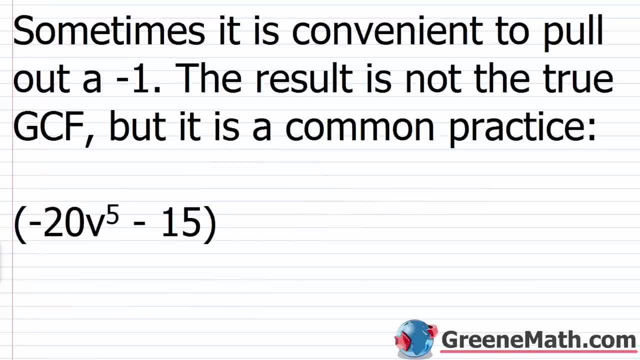 So sometimes it is convenient to pull out a negative 1. The result is not the true GCF, but it's common practice. 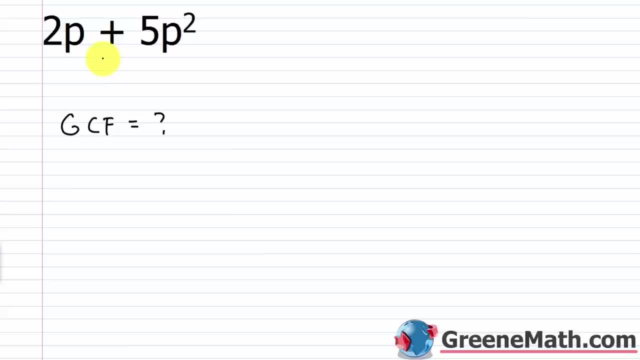 would just be the number 1.. So kind of moving on, we see that they each have the variable p. 1 is p to the first power. 1 is p squared, So you use the exponent on the variable that's smallest. 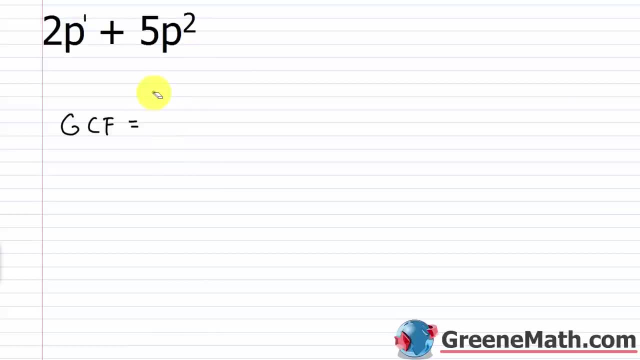 In this case that's going to be 1.. So the greatest common factor is just p. Alright, so to factor this guy out again, I'm going to put p outside of a set of parentheses. So inside what am I going to use to fill these? 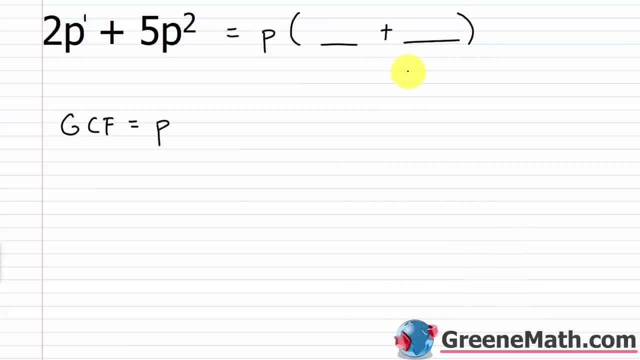 two spaces. Again, I can do it two ways. I can divide 2p by p, 2p by p, That's going to give me 2.. And then I can divide 5p squared by p, That's going to give me. 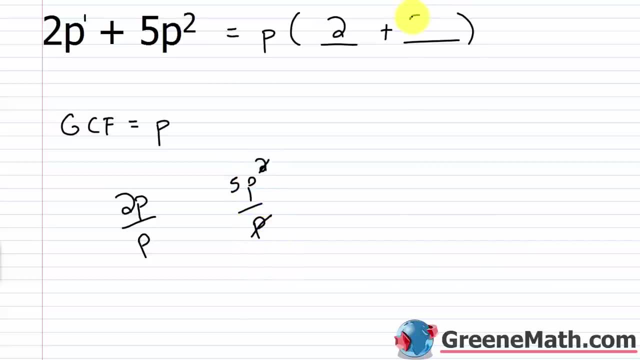 this will cancel with this 5p, So 5p And then the other way again. if you're more comfortable doing it this way, you could also say: okay, well, I have 2 times p. I'm going to write this in a different. 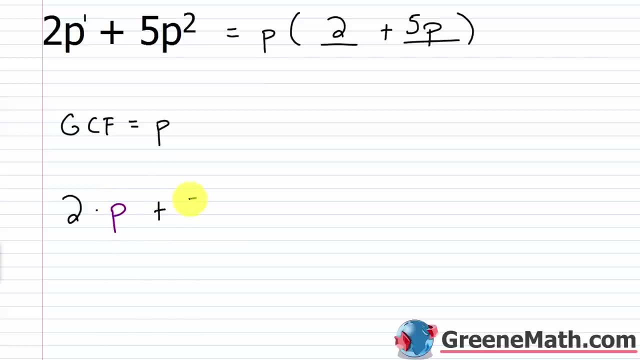 color, And then plus I have 5 times p times p. So then it makes it completely obvious that I'm going to pull this out in each case. pull this out, place it outside of the parentheses and then what's left. So I'd have a 2 here. 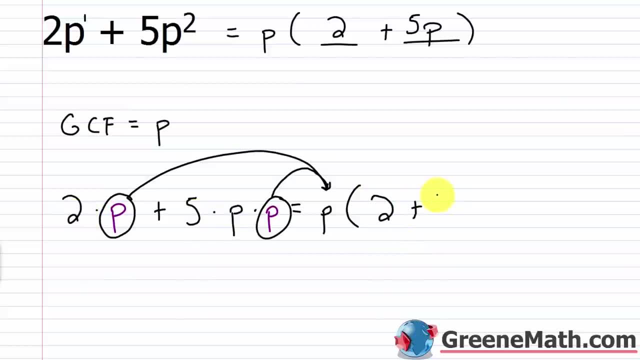 plus in here, I'd have 5p. So either way you want to do it, you would get p times the quantity 2 plus 5p. And if it makes you feel more comfortable, because I know none of this is in standard form- 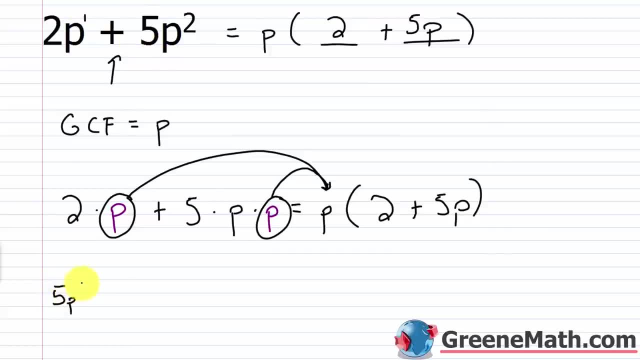 you could flip the order of this to begin. So you could say: 5p squared plus 2p is equal to, and then you'd have p times flip the order of this: 5p plus 2.. And again you can check it with multiplication. 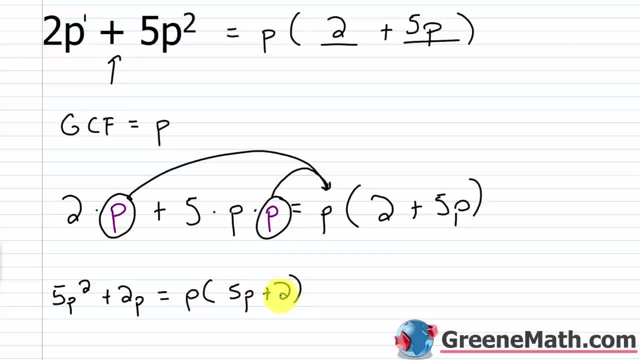 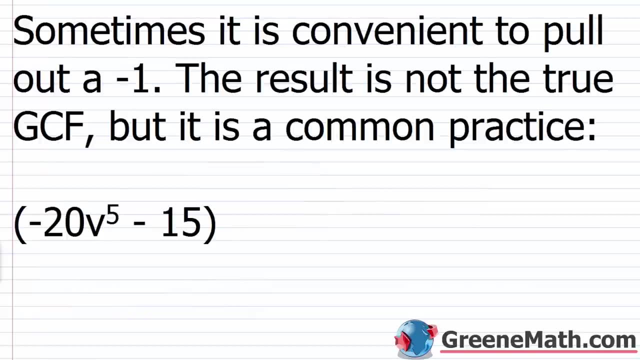 p times 5p is 5p. squared p times 2 is 2p, So you'd get 5p squared plus 2p, Alright. so here's another thing that trips students up a lot, So sometimes it is convenient. 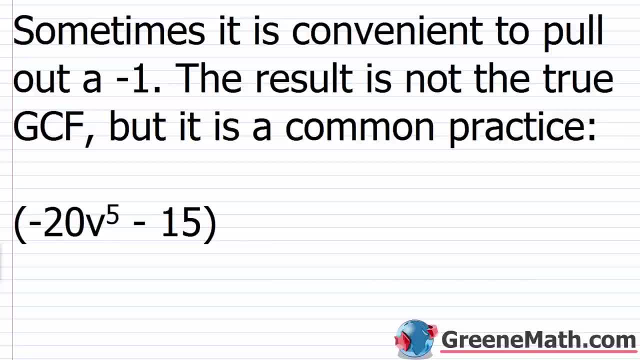 to pull out a negative 1. The result is not the true GCF but it's common practice. So your teacher might say on the instructions to pull out the greatest common factor. but it might be more convenient for you to pull out a. 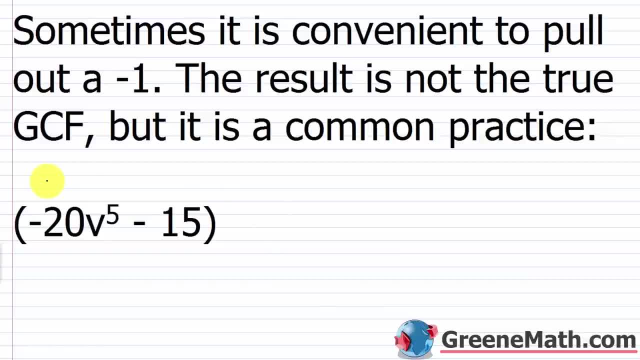 negative 1. And this might not result in this section but kind of moving forward in the next section. when we start talking about factoring by grouping, you're going to see right away that sometimes you have to pull out the negative of the GCF to get everything to work. 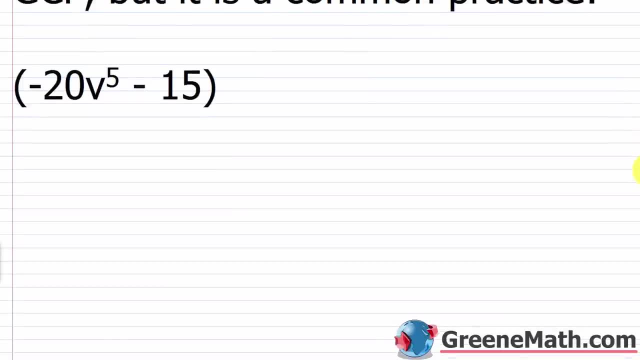 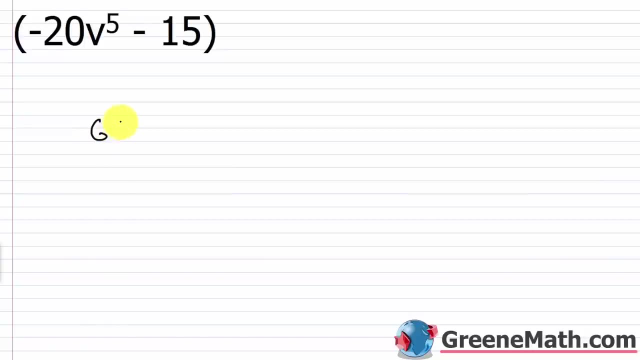 out. So let's take a look at this real quick. So I have negative 20v to the fifth, power minus 15.. So what is the GCF here, The greatest common factor? Well, if I look at negative 20v to the fifth, 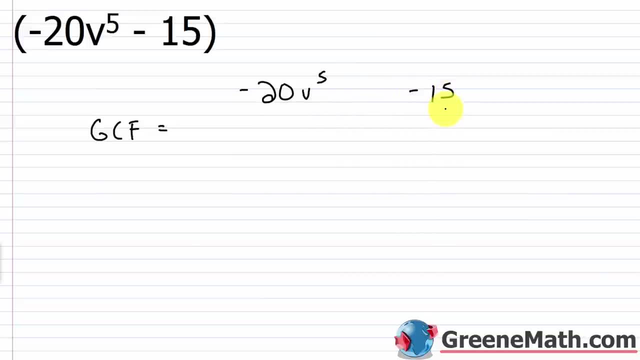 power and I look at negative 15, I know there's no variable involved, so I can really write negative 20 as negative 1 times, 5 times, let's just say 4. Let's shorten it a little bit. And negative 15 I can write as: 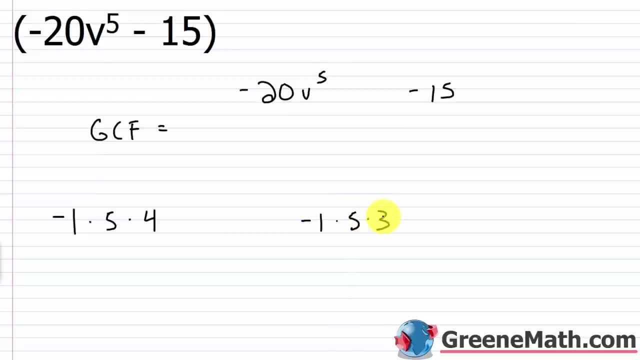 negative 1 times 5 times 3.. So the GCF, the greatest common factor between the two, is 5.. So let's start out by doing it with that, And then we're going to try negative 5. Because we have a common factor of negative. 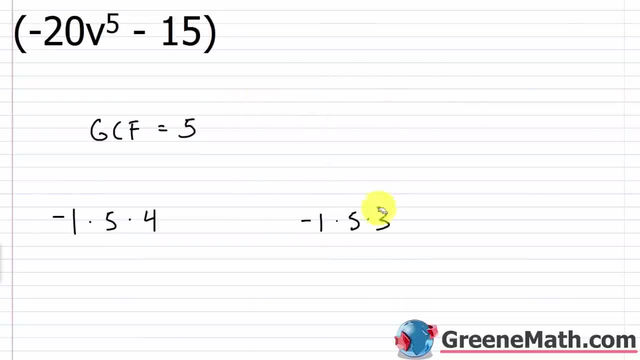 1 between the two, So let's start out with just 5.. So this is equal to: I'm going to put my greatest common factor out in front and I have my parentheses: space minus space. Okay, So if I took negative, 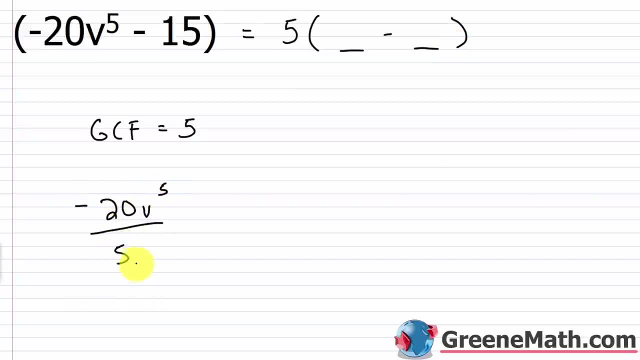 20v to the fifth power and I divide it by 5, this would cancel with this and I'd have negative 4.. So I'd have negative 4 v to the fifth power, Then minus. Next I'd have 15 divided by 5,. 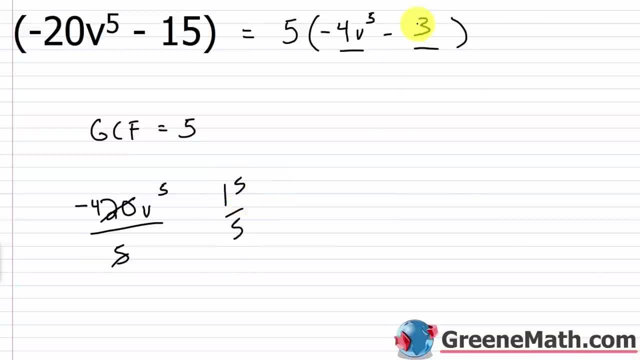 and we know that's 3.. We know that's 3.. So that's factoring out the greatest common factor. But again, sometimes you might not want to do that. Sometimes you might want to factor out a negative 5 because you might not want minus signs in here. 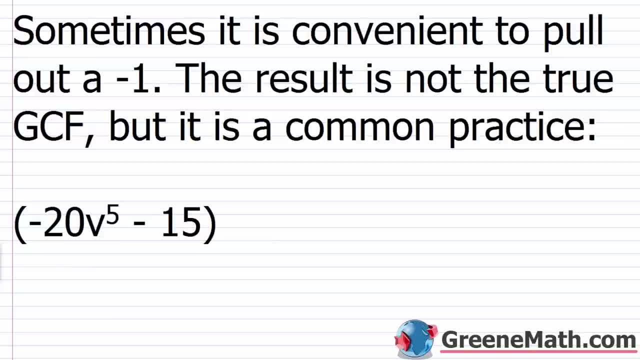 So your teacher might say on the instructions to pull out the greatest common factor, but it might be more convenient for you to pull out a negative 1. 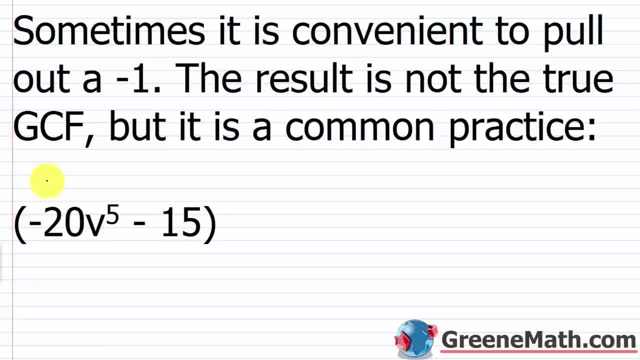 And this might not result in this section, but kind of moving forward, in the next section, when we start talking about factoring by grouping, you're going to see right away that sometimes you have to pull out the negative of the GCF to get everything to work out. So let's take a look at this real quick. 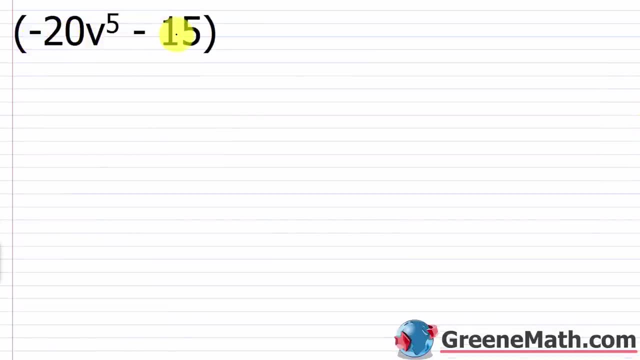 So I have negative 20v to the fifth power minus 15. So what is the GCF here? The greatest common factor. Well, if I look at negative 20v to the fifth power, and I look at negative 15, I know there's no variable involved, so I can really write negative 20 as negative 1 times 5 times, let's just say 4, let's shorten it a little bit. 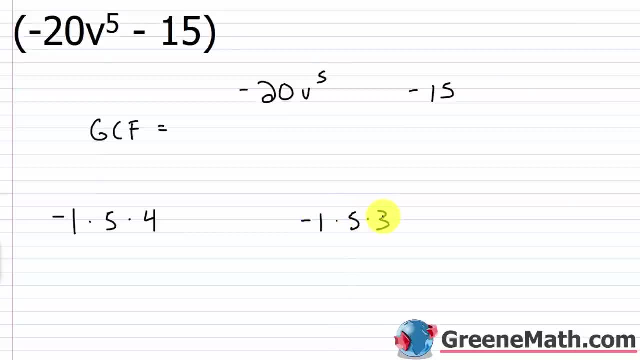 And negative 15 I can write as negative 1 times 5 times 3. 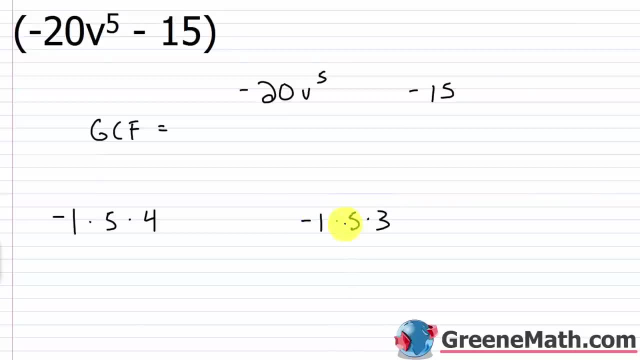 So the GCF, the greatest common factor between the two, is 5. 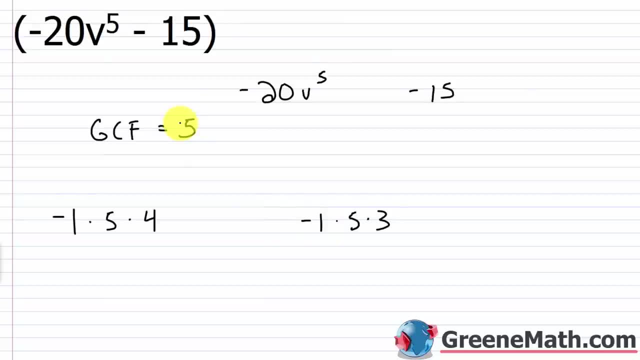 So let's start out by doing it with that. And then we're going to try negative 5, because we have a common factor of negative 1 between the two. So let's start out with just 5. 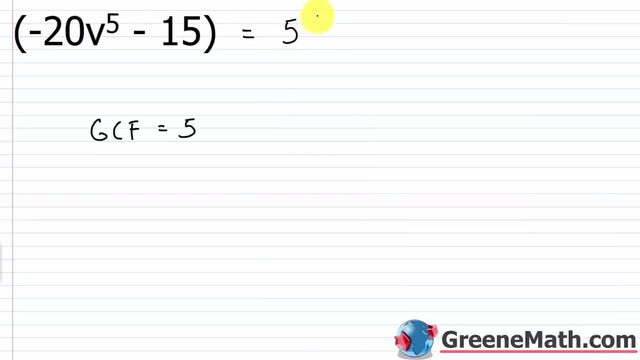 So this is equal to, I'm going to put my greatest common factor out in front, and I have my parentheses, space, minus, Okay. 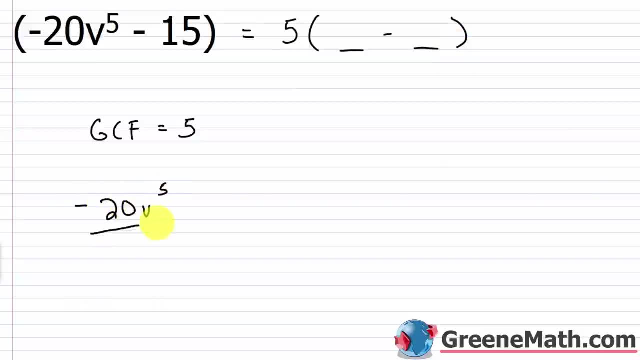 So if I took negative 20v to the fifth power, and I divide it by 5, this would cancel with this, and I'd have negative 4. 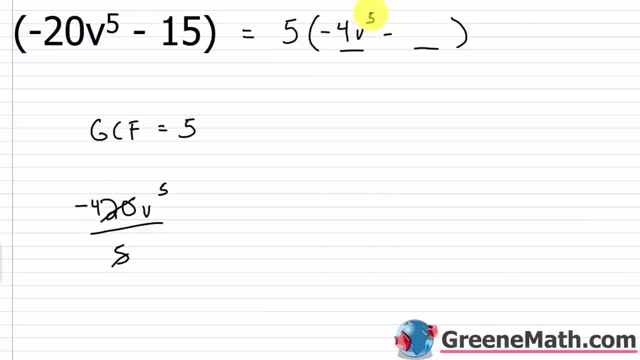 So I'd have negative 4v to the fifth power, then minus. Next I'd have 15 divided by 5, and we know that's 3. We know that's 3. 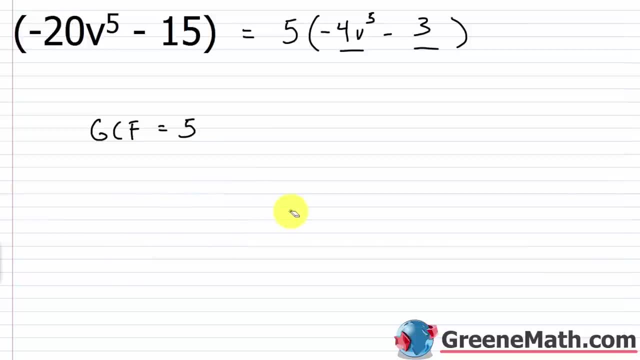 So that's factoring out the greatest common factor. But again, sometimes you might not want to do that. 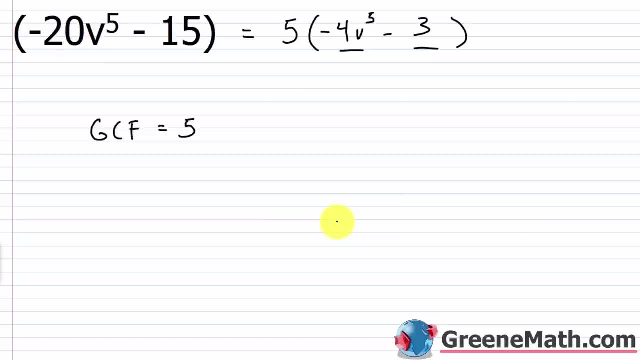 Sometimes you might want to factor out a negative 5, because you might not want minus signs in here. Right? 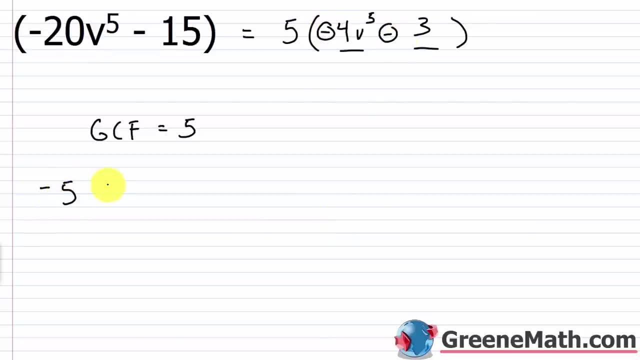 So if I factored out a negative 5, what would I have then? Well, if I think about this, negative 20 divided by negative 5 is positive 4. Then I have v to the fifth power. Negative 15, I'm going to include that sign there, 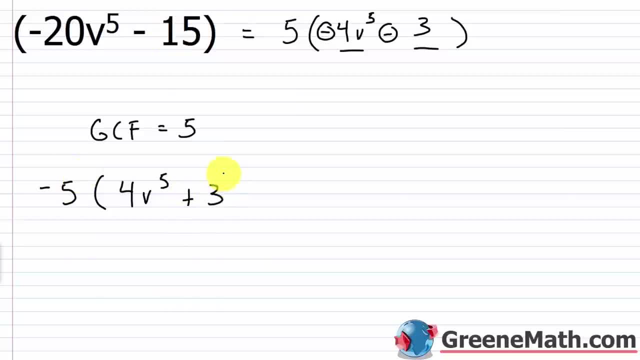 negative 15 divided by negative 5 is plus 3. 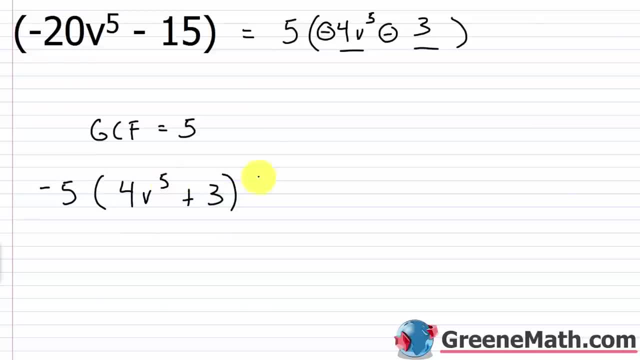 So either way you do it, if you went back and used your distributive property, you get this back. 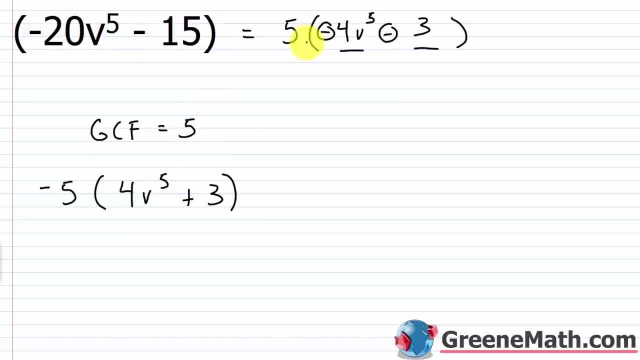 But by definition, 5 is the greatest common factor. So this would be the true answer. But again, in some cases, you're going to need to factor out the negative of the GCF. 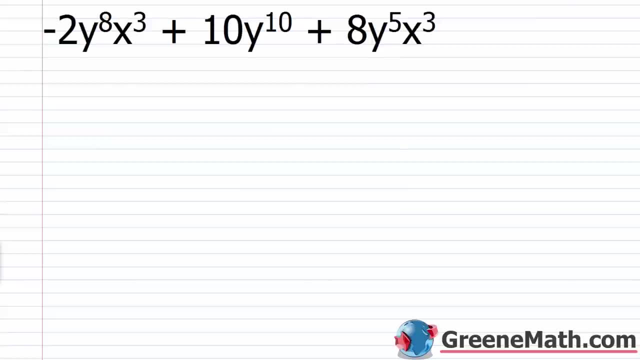 And so you'd want to do it this way. All right, let's take a look at another one. 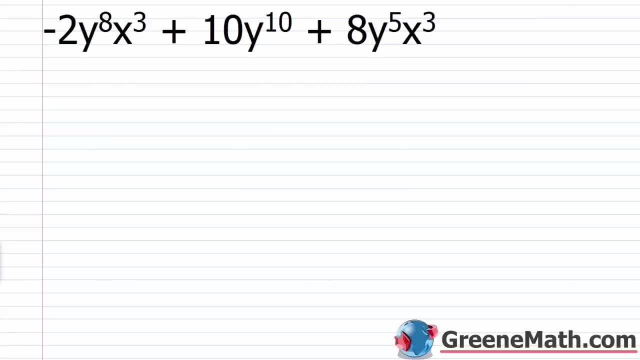 We have negative 2y to the eighth power x cubed, plus 10y to the 10th power, plus 8y to the fifth power x cubed. 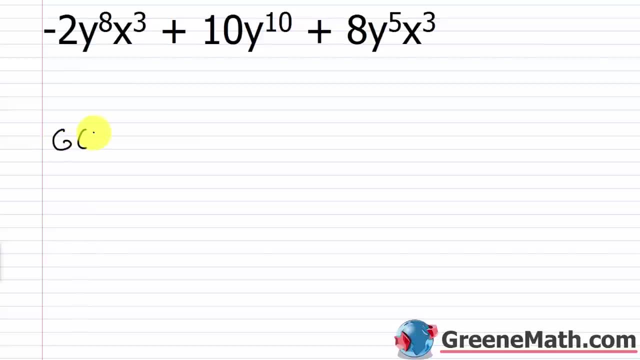 Okay. So what is the greatest common factor here? Well, 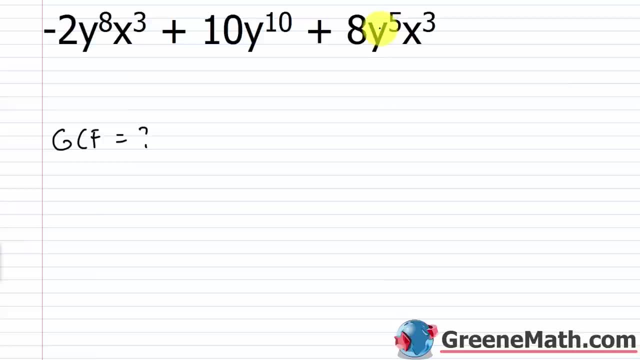 I know that there's a y in each term, but there's not an x in each term. 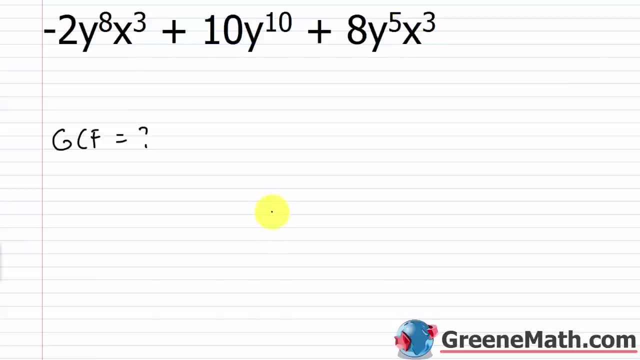 So x won't be involved. The variable part is pretty easy. 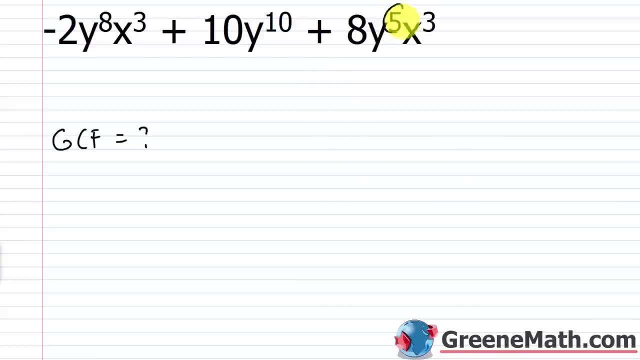 The lowest exponent on any of the variables is a 5. So that'd be y to the fifth power. And then as far as the numbers go, each one is divisible by 2. 2 is the smallest number. So, it's a prime number. And it's a prime number. 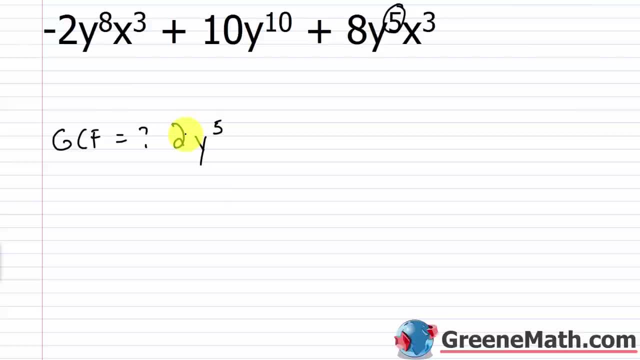 So it's going to be 2y to the fifth power. So I'm going to pull that guy out. I'm going to have 2y to the fifth power. And that's going to be times, I'm going to have three spaces here, because I have three terms. So again, I can just divide each. 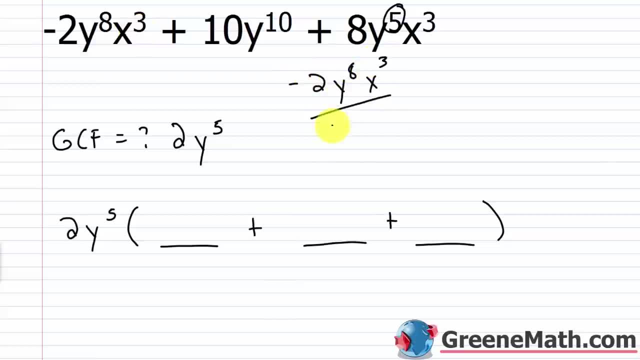 So negative 2y to the eighth power x cubed, divided by 2y to the fifth power. Negative 2 over 2 is negative 1. So I'll just put a negative out in front. Then y to the eighth over y to the fifth is y cubed. 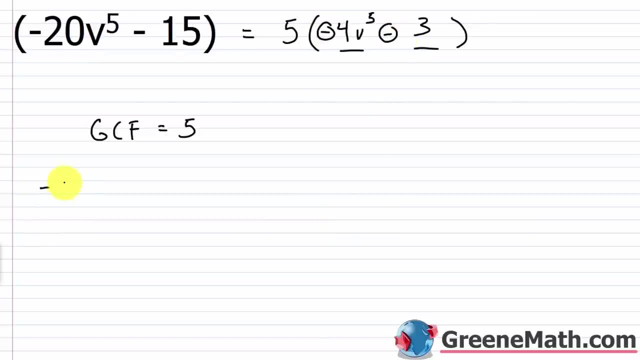 Right. So if I factored out a negative 5, what would I have then? Well, if I think about this, negative 20 divided by negative 5 is positive 4.. Then I have v to the fifth power, Negative 15, I'm going to include: 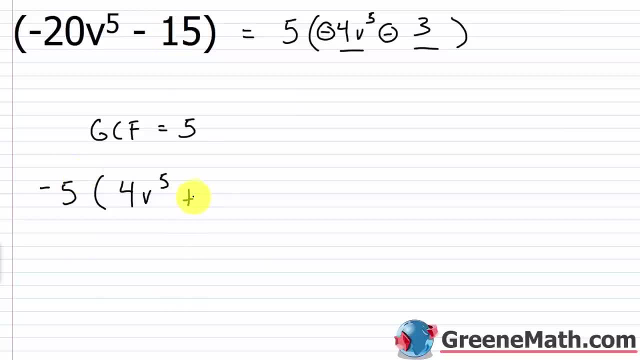 that sign there. negative 15 divided by negative 5 is plus 3.. So either way you do it, if you went back and used your distributive property you get this back. But by definition, 5 is the greatest common factor. so this would: 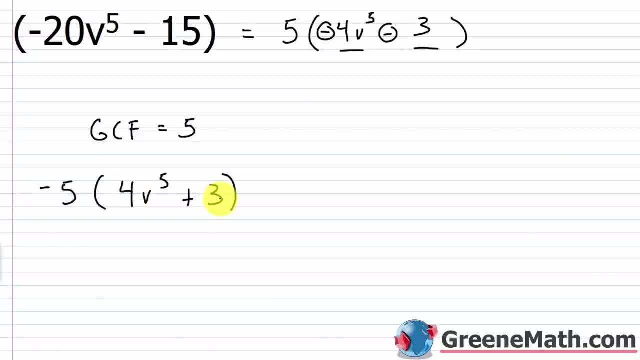 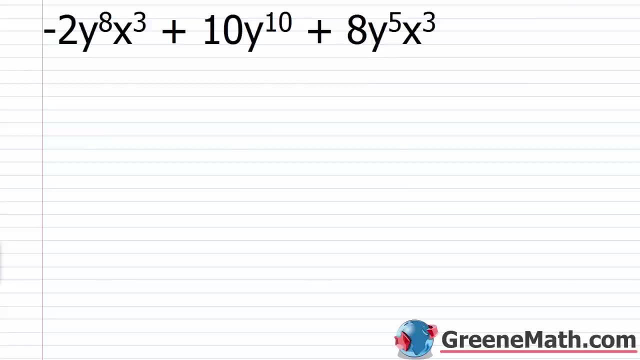 be the true answer. But again, in some cases you're going to need to factor out the negative of the GCF, and so you'd want to do it this way. Alright, let's take a look at another one. We have negative 2y to the eighth power. 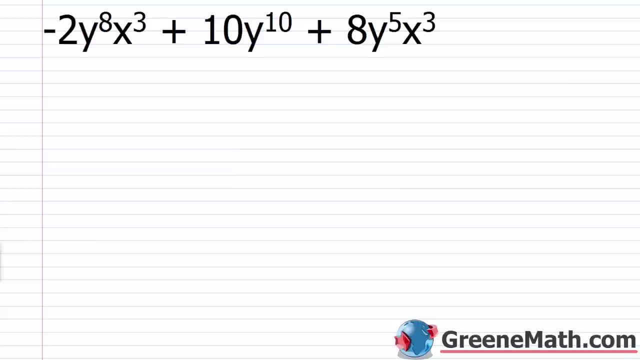 x cubed, plus 10y to the tenth power, plus 8y to the fifth power- x cubed. Okay, So what is the greatest common factor here? Well, I know that there's a y in each term, but there's not an x. 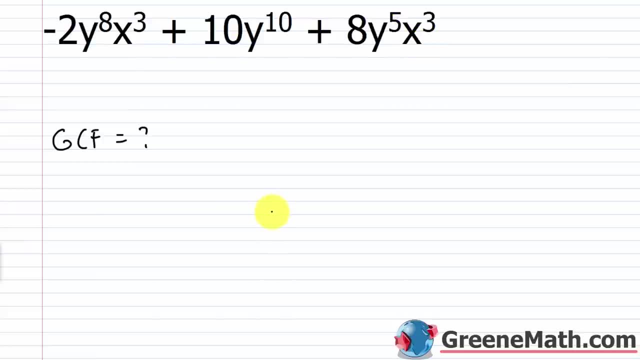 in each term, so x won't be involved. The variable part is pretty easy. The lowest exponent on any of the variables is a 5, so that would be y to the fifth power, And then, as far as the numbers go, each one is divisible by: 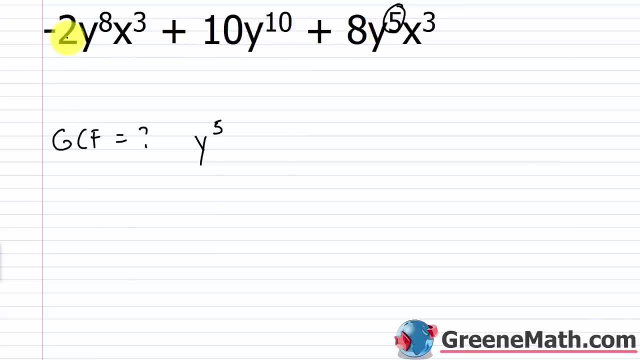 2.. 2 is the smallest number and it's a prime number, so it's going to be 2y to the fifth power. So I'm going to pull that guy out. I'm going to have 2y to the fifth power. 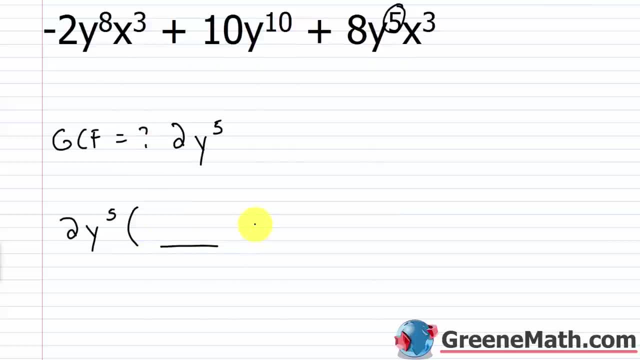 And then it's going to be times. I'm going to have three spaces here because I have three terms, So again I can just divide each. so negative 2y to the eighth power, x cubed divided by 2y to the fifth power. 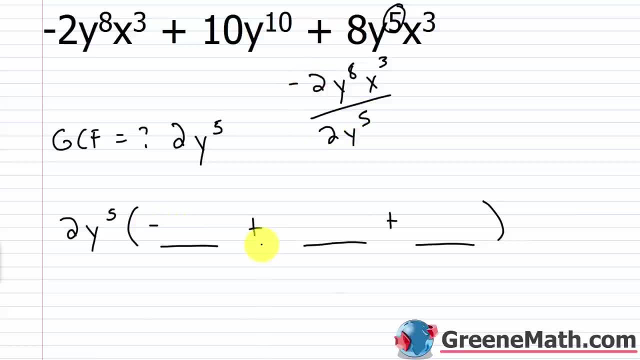 Negative 2 over 2 is negative 1, so I'll just put a negative out in front. Then y to the eighth over y to the fifth is y cubed, And then x cubed is just going to come along for the ride here. 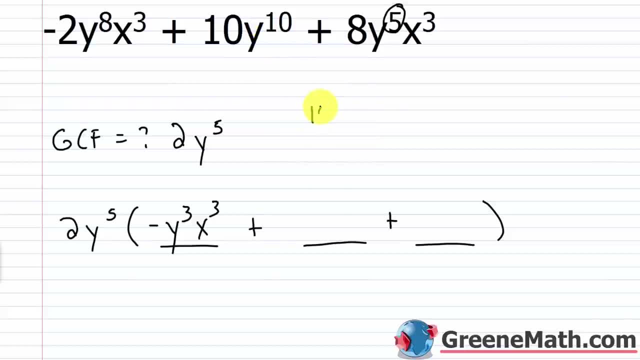 Alright, let me erase this Kind of move to the next term. You'd have 10 y to the tenth over 2 y to the fifth. 10 over 2 is 5.. y to the tenth over y to the fifth is y to the fifth. 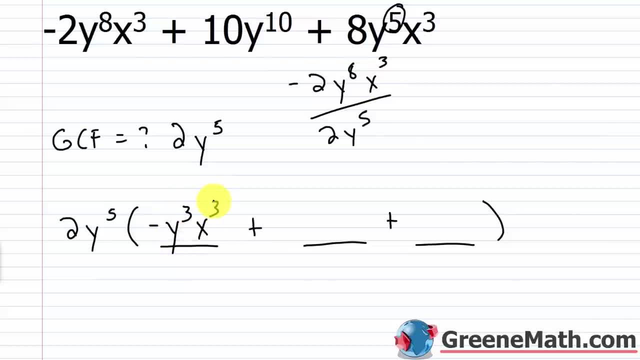 And then x cubed is just going to come along for the ride here. All right, let me erase this. Kind of move to the next term. 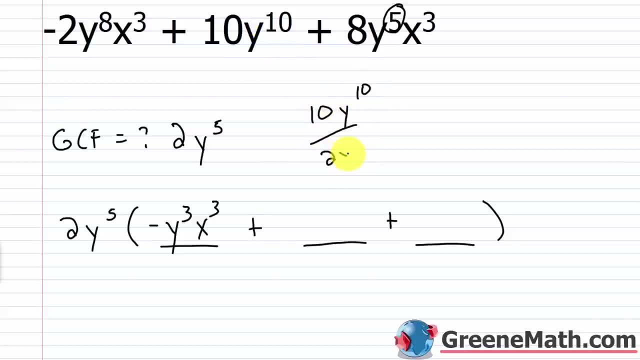 You'd have 10y to the tenth over 2y to the fifth. 10 over 2 is 5. 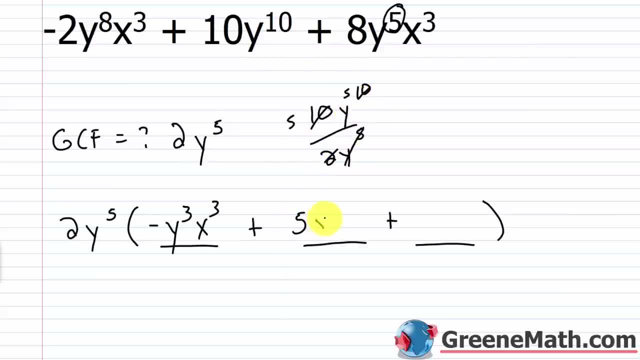 y to the tenth over y to the fifth is y to the fifth. 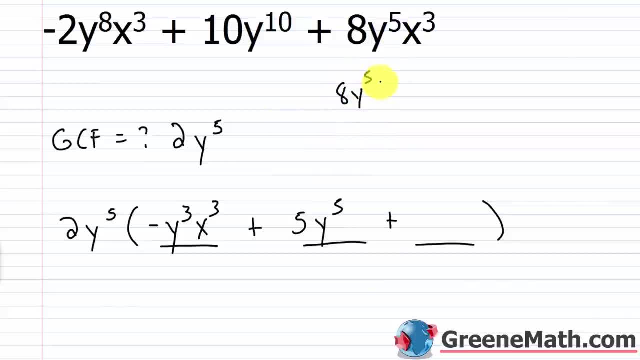 All right, for kind of the last term here, we have 8y to the fifth power x cubed. This is over 2y to the fifth power. 8 over 2 is 4. y to the fifth over y to the fifth is 1. 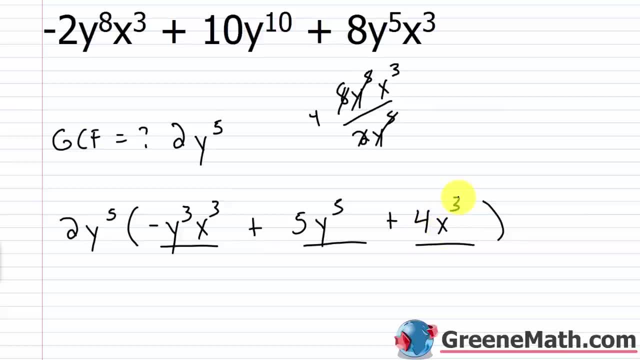 So you would get 4x cubed. And so we have our answer here. In factored form, this is 2y to the fifth power, times the quantity negative y cubed x cubed, 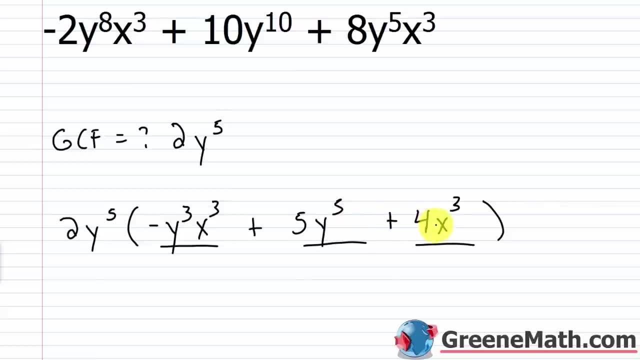 plus 5y to the fifth power plus 4x cubed. 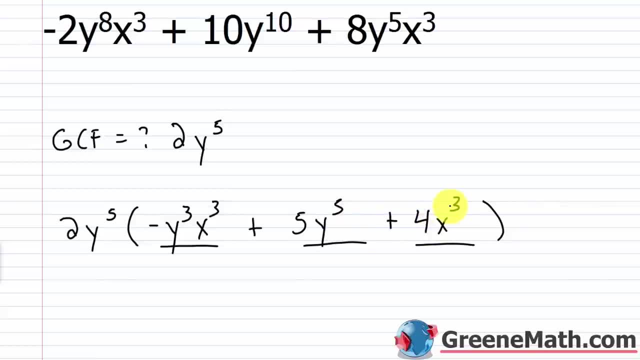 Now, again, you might come across a situation where, you want to factor out the negative of the GCF. 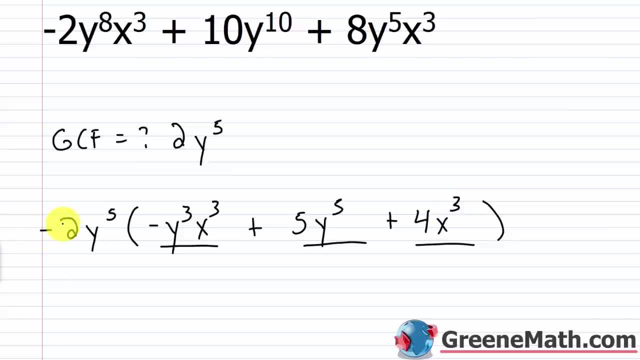 So if I factored out a negative 2y to the fifth power, all the signs in here would just change, right? So if I multiply or divide by a negative, it just changes the sign. So this would be plus, this would be minus, this would be minus, right? But again, if I change this back to plus, then this becomes minus plus plus. 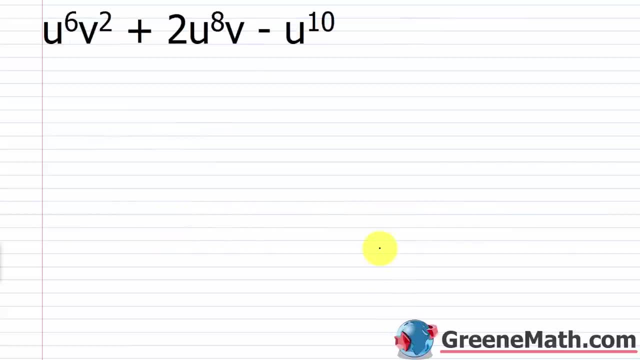 So for the next one, I have u to the sixth power v squared, plus 2u to the eighth power v squared, minus u to the tenth power. 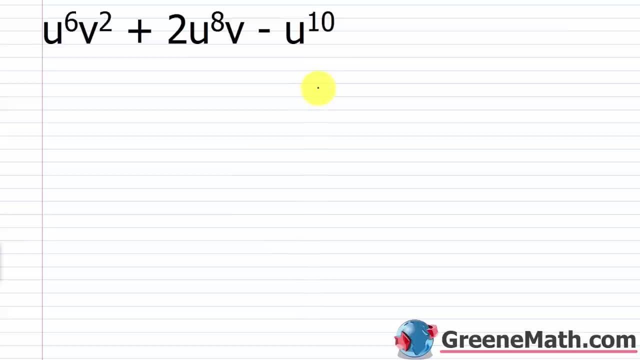 So what is my GCF here? There's obviously not going to be any numbers involved. 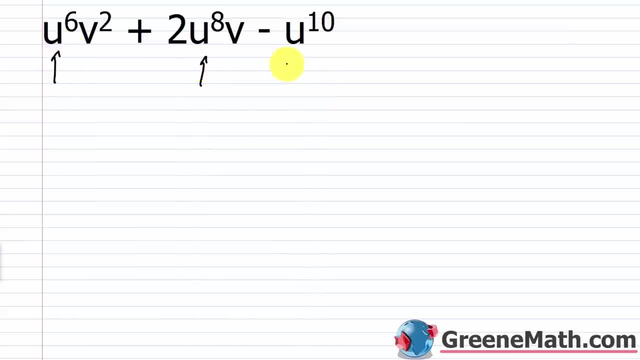 I have u to the sixth power, u to the eighth, and u to the tenth. A v is not going to be involved, because it's not common to everything. 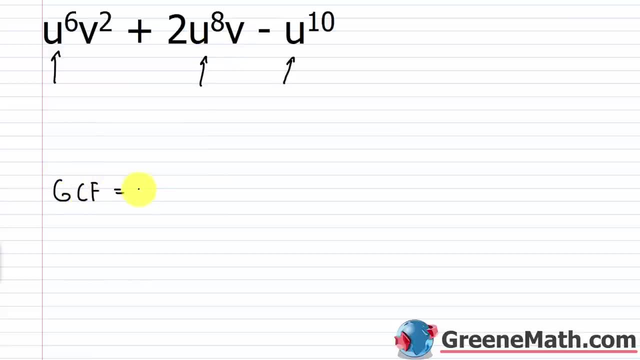 So my GCF here, my GCF is u to the sixth power. So let's pull that out. So let's pull that out. And what's going to be left? Well, 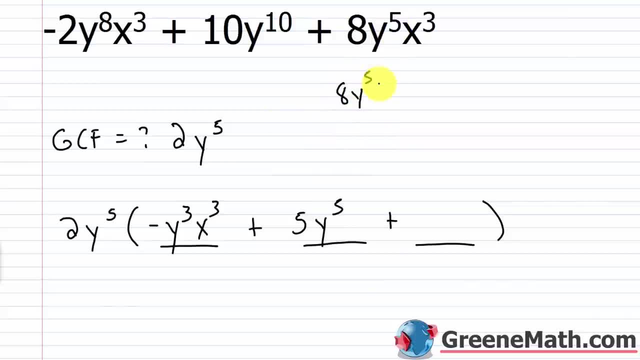 Alright, for kind of the last term. here we have 8y to the fifth power, x cubed. This is over 2y to the fifth power. 8 over 2 is 4.. y to the fifth over y to the fifth is 1.. 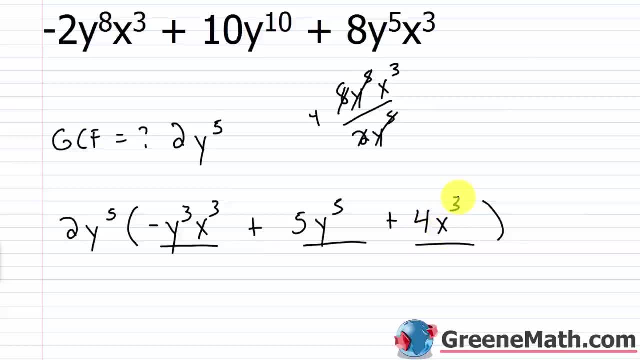 So you would get 4x cubed, And so we have our answer here In factored form. this is: 2y to the fifth power times the quantity negative y cubed, x cubed plus 5y to the fifth power plus 4x cubed. 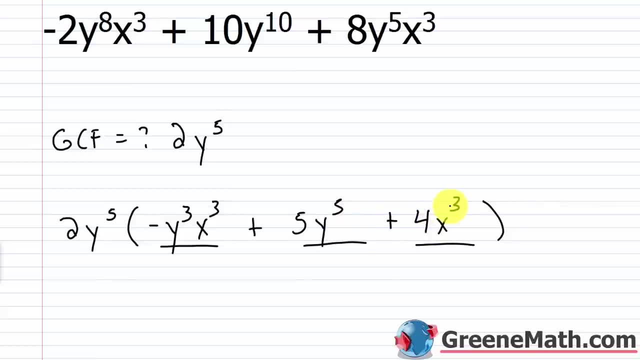 Now again, you might come across a situation where you want to factor out the negative of the GCF. So if I factored out a negative 2y to the fifth power, all the signs in here would just change. Alright, so if I multiply, 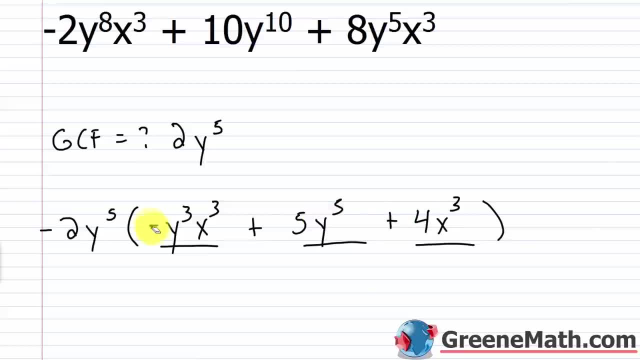 or divide by a negative. it just changes the sign. So this would be plus, this would be minus, this would be minus. But again, if I change this back to plus, then this becomes minus, plus, plus. So for the next one, I have u to the sixth power. 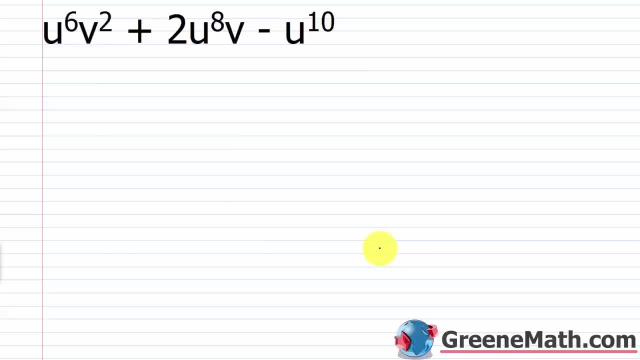 v squared plus 2u to the eighth power, v minus u to the tenth power. So what is my GCF here? There's obviously not going to be any numbers involved. I have u to the sixth power, u to the eighth and u to. 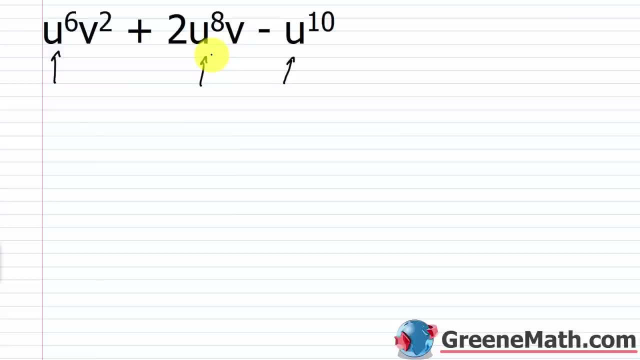 the tenth A v is not going to be involved because it's not common in everything. So my GCF here, my GCF, is u to the sixth power. So let's pull that out. So let's pull that out. And what's going to be left? Well, if I have, 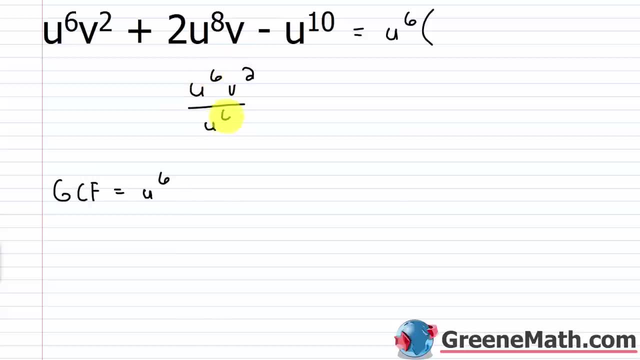 u to the sixth power, v squared over u to the sixth power. this is going to cancel and I'll just have v squared If I have 2u to the eighth power, v over u to the sixth power. this is going to cancel. with this, I'll have. 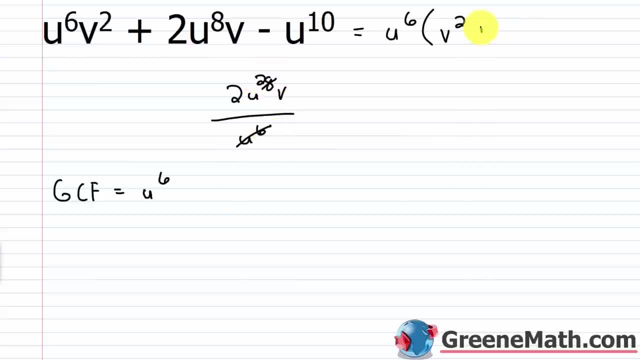 u to the second power or u squared. So this will be plus 2u to the second power, v Then minus. if I have u to the tenth power, u to the tenth power over u to the sixth power, we're going to cancel this out. 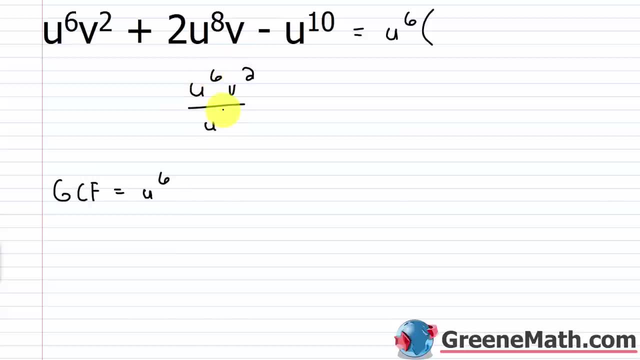 if I have u to the sixth power v squared, over u to the sixth power, this is going to cancel, and I'll just have v squared. 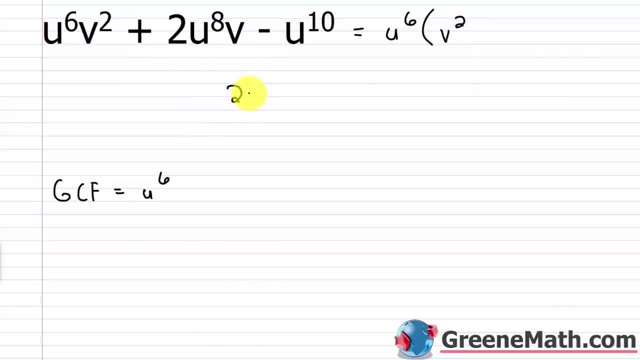 If I have 2u to the eighth power v, over u to the sixth power, this is going to cancel with this. I'll have u to the second power, or u squared. 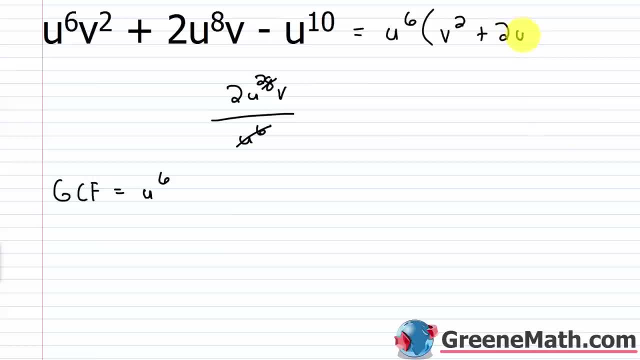 So this will be plus 2u to the second power v. Then minus, if I have u to the tenth power, u to the tenth power, over u to the sixth power, over u to the sixth power, we're going to cancel this out, and this will be a four. 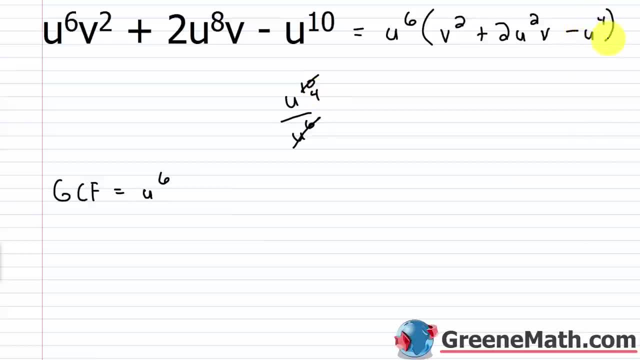 So this will be u to the fourth power. And so I'd have my answer, u to the sixth power times the quantity, v squared plus 2u squared v, minus u to the fourth power. All right, let's take a look at another one. 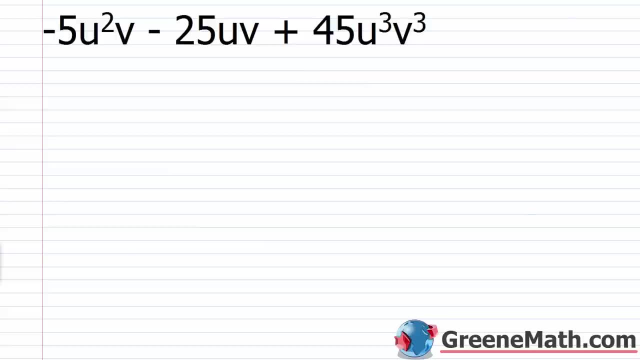 We have negative 5u squared v, minus 25uv, plus 45u cubed v cubed. 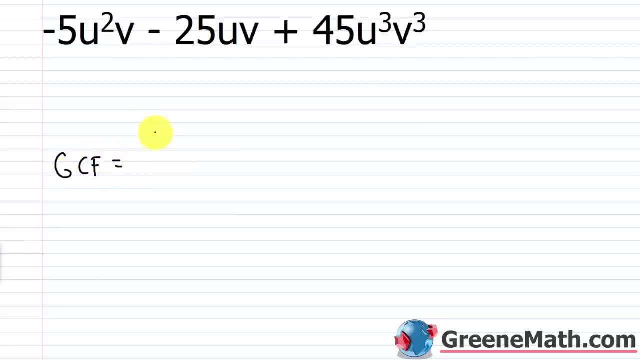 So my GCF here, if you look at the number parts, it's going to be 5, right? You have 5 here. 25 is 5 times 5. 45 is 5 times 9. 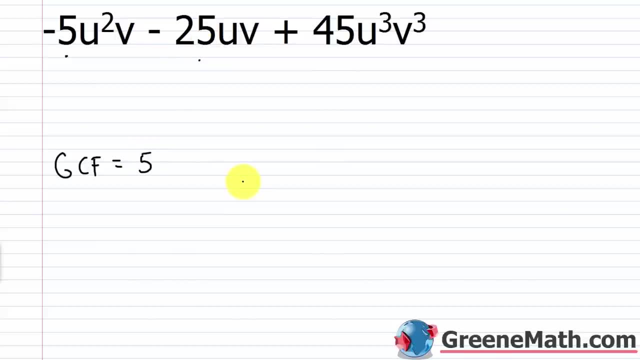 So it's going to be 5. And then for the variable part, you have a u in each case, and you have a v in each case. The smallest exponent on each is a 1, so it'll be uv. Okay. 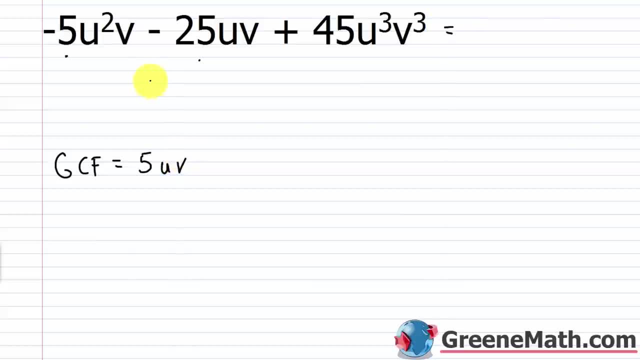 So if we want to pull this guy out, let me write this down here, you'd have 5uv, outside of parentheses. So I'm going to divide each term here by this. 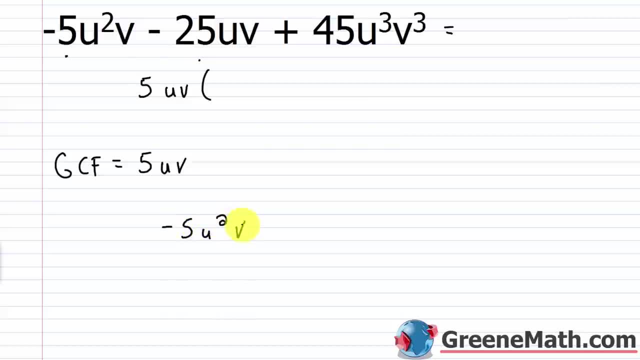 So negative 5u squared v over 5uv. We know that negative 5 over 5 is negative 1. u squared over u, this is going to cancel, be u to the first power. v over v is 1. So you'd have a negative u, basically. 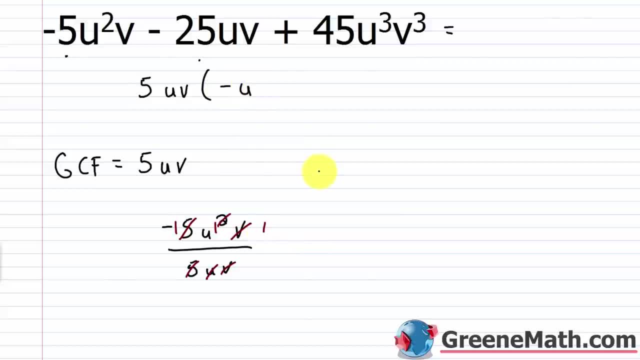 Negative u. And then you would have minus. We have 25, 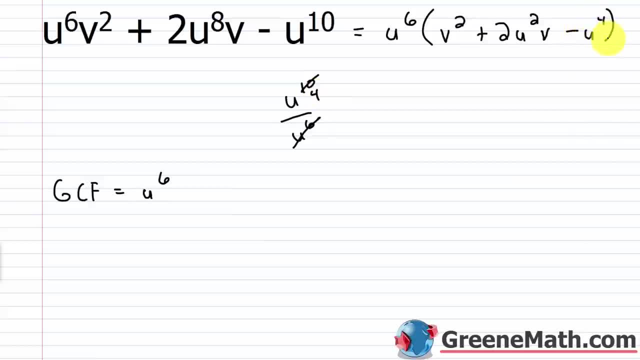 and this will be a 4.. So this will be u to the fourth power, And so I'd have my answer: u to the sixth power times the quantity b squared plus 2u, squared v minus. u to the fourth power. Alright, let's take a look at another one. 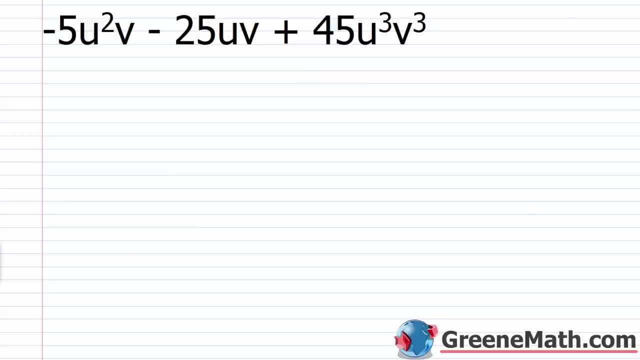 We have negative 5u squared v minus 25uv plus 45u cubed v cubed. So my GCF here. if you look at the number parts, it's going to be 5.. You have 5 here. 25 is. 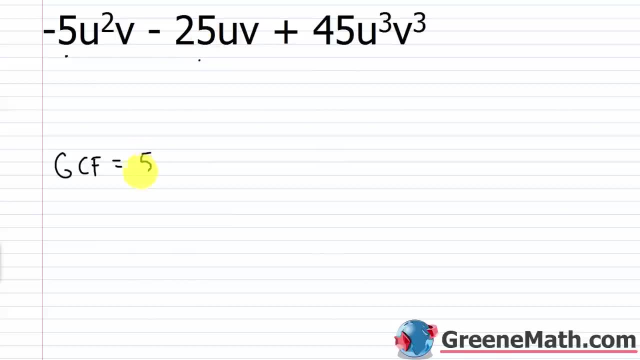 5 times 5, 45 is 5 times 9.. So it's going to be 5.. And then, for the variable part, you have a u in each case and you have a v in each case. The smallest exponent on each is a 1.. 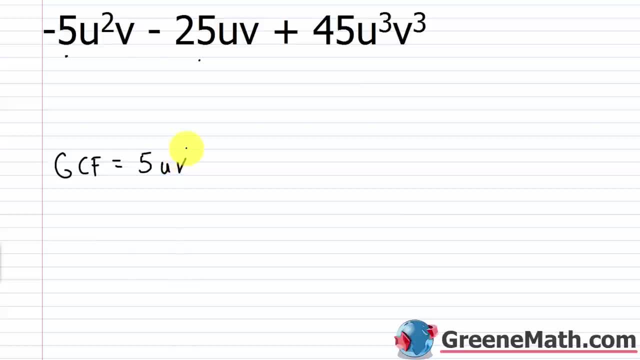 So it'll be uv. Okay. So if we want to pull this guy out, let me write this down here: you'd have 5 uv outside of parentheses, So I'm going to divide each term here by this. So negative 5. 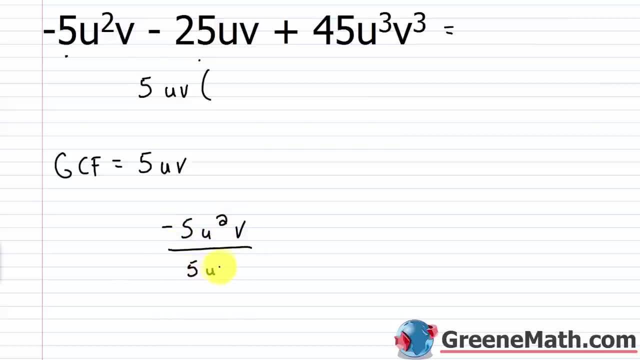 u squared v over 5uv. We know that negative 5 over 5 is negative 1.. u squared over u. this is going to cancel. be u to the first power. v over v is 1.. So you'd have a. 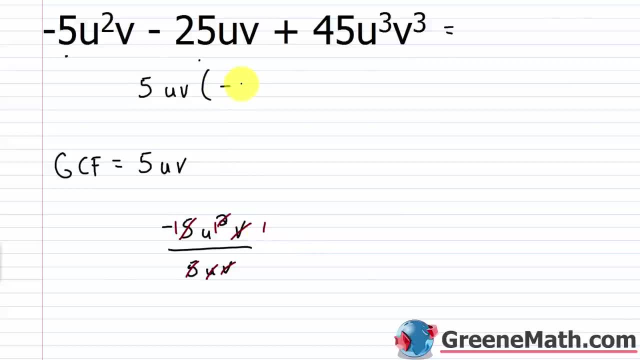 negative u, basically Negative u, And then we have minus, We have 25.. 25uv over 5uv, So the uv in each case is going to cancel. 25 over 5 is 5.. So this is minus 5. 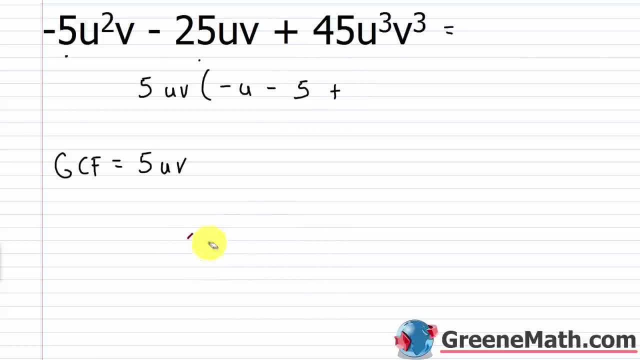 here and then plus Next, we have this 45. Again, 45 u cubed v over 5 uv. So then 45 over 5 is 9.. u cubed over u is u squared v. cubed over v is v. 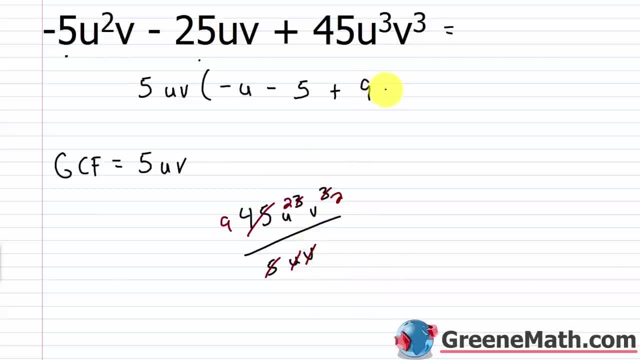 squared, So this is going to end up being 9u squared v squared. Okay, So that's my answer: 5uv times the quantity negative: u minus 5 plus 9u squared v squared. Now again, I want to come back to the 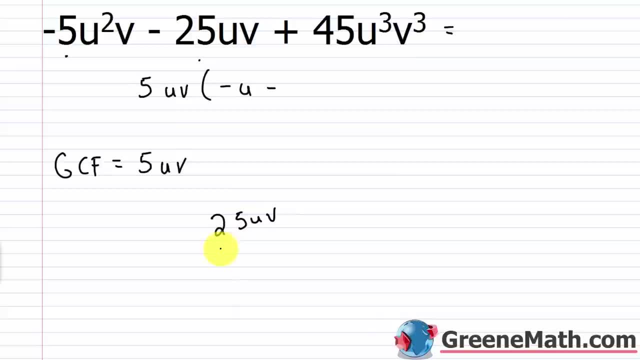 25uv, over 5uv. So the uv in each case is going to cancel. 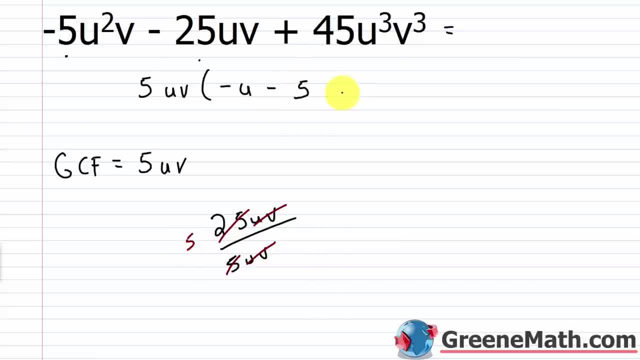 25 over 5 is 5. So this is minus 5 here, and then plus. 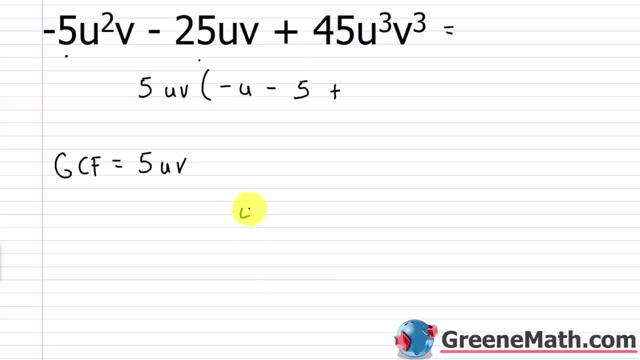 Next we have this 45. Again, 45u cubed v cubed over 5uv. So then 45 over 5 is 9. u cubed over u is u squared. v cubed over v is v squared. So this is going to end up being 9u squared v squared. So that's my answer. 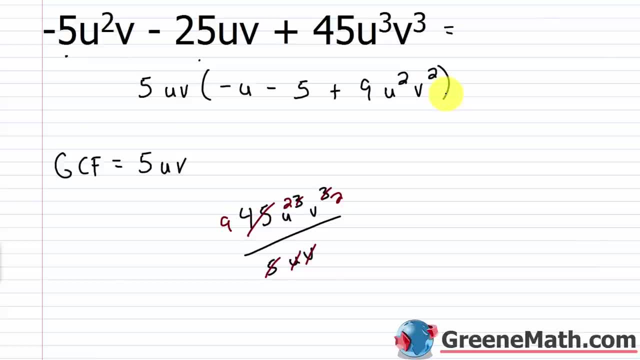 5uv times the quantity negative u minus 5 plus 9u squared v squared. 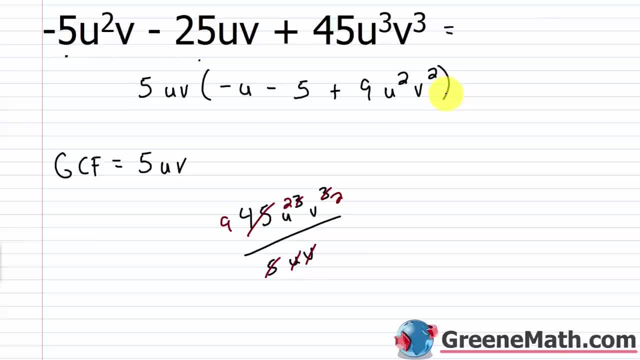 Now, again, I want to come back to the fact that we can also do the negative of the GCF. Let me show you a little trick for this. One other way you can do it. 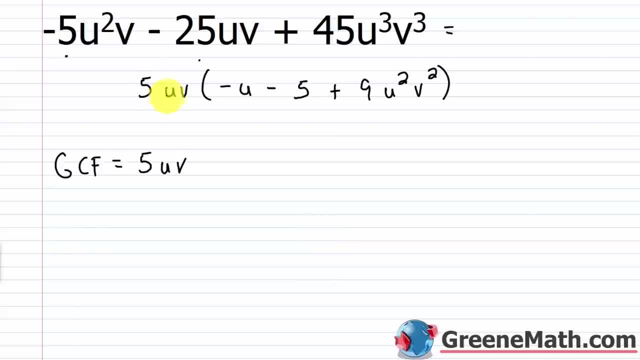 So let's say I decided to factor out a negative 1 times 5uv. So let's write this as negative 1 times 5 times u times u times v. And then instead of minus, I'm going to put plus. 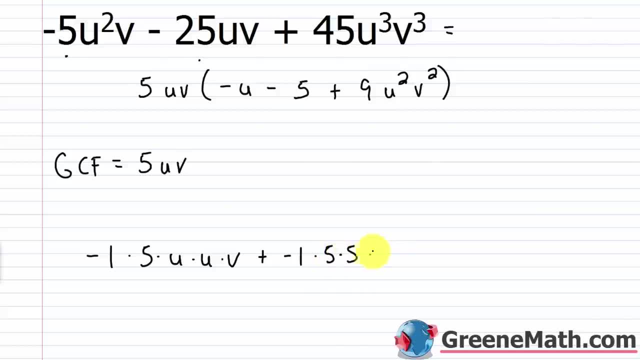 I'm going to put negative 1 times 5 times 5 times u times v. And then plus. One more time. Instead of 45, what can I write? 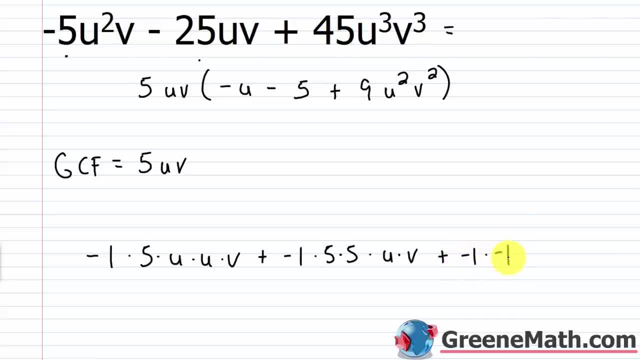 I can write negative 1 times negative 1. Negative 1 times negative 1 is positive 1. So I'm not really doing anything illegal. So I'm just going to write 1 times 5 times 9. 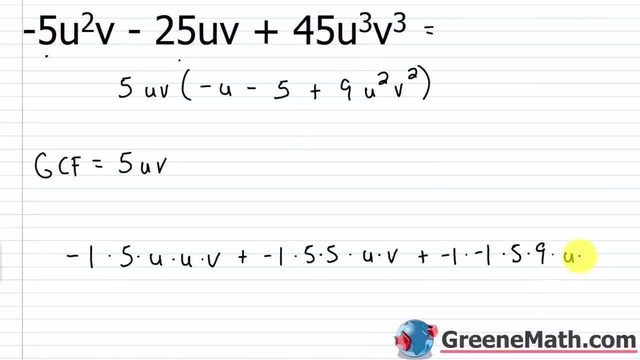 And then I need a little bit more room. So times u times u times u. 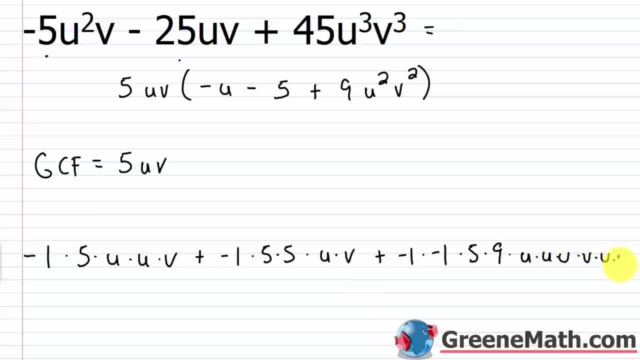 Let me move this over a little bit. And then times v times v times v. Okay. 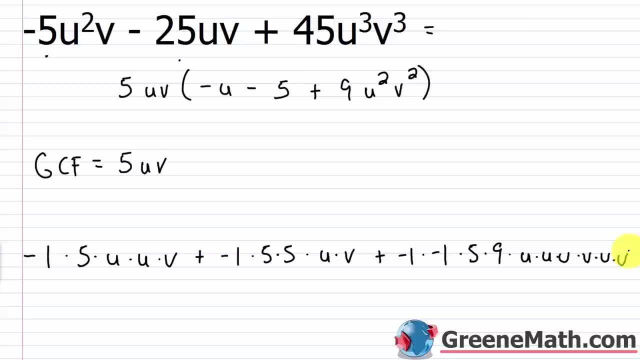 So if I look at the negative of the GCF, that's negative 5. So that's negative 5. 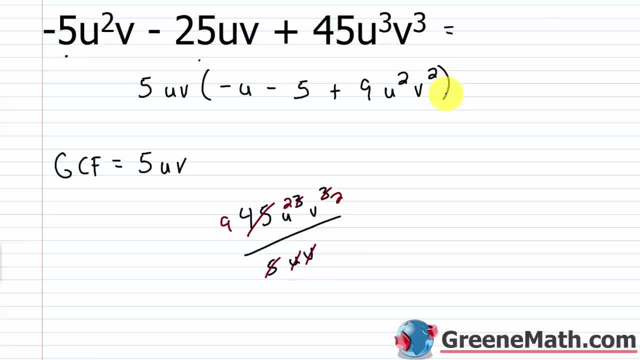 fact that we can also do the negative of the GCF. Let me show you a little trick for this, One other way you can do it. So let's say I decided to factor out a negative 5uv, So let's write this as negative 1. 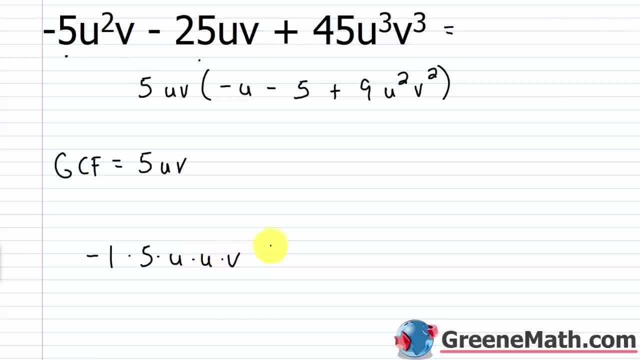 times 5 times u times u times v. And then, instead of minus, I'm going to put plus. I'm going to put negative 1 times 5 times 5 times u times v, And then plus One more time instead of 45. 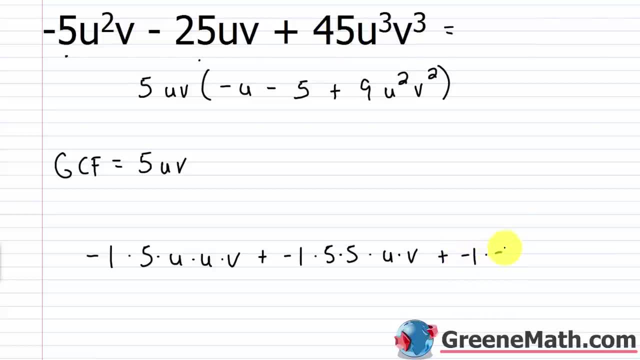 what can I write? I can write negative 1 times negative, 1. Right Negative 1 times negative, 1 is positive, 1. So I'm not really doing anything illegal. Then times 5 times 9.. And then I need a little. 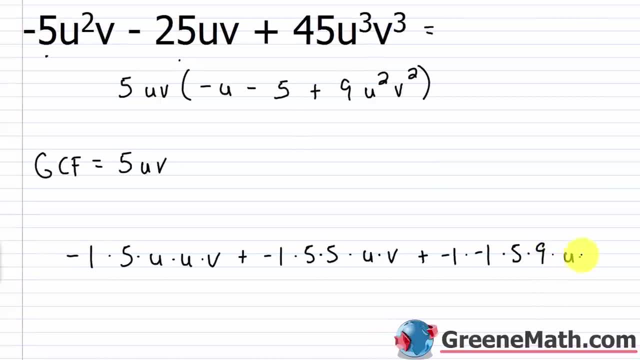 bit more room. So times u, times u, times u. I'm going to move this over a little bit And then times v, times v, times v. Okay, So if I look at the negative of the GCF, that's negative 5.. 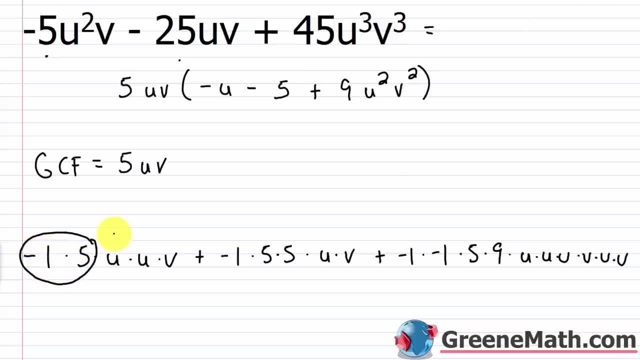 So that's negative 5.. And then for the variable part it's uv. So I'm going to circle that in each case Negative 5, uv, So negative 5 and then uv. So if you think about it here, what would be left? 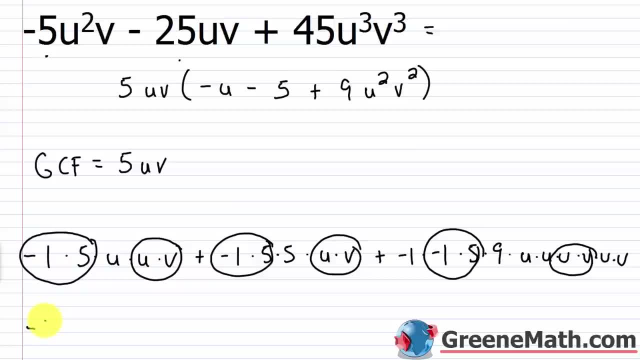 If I pulled out the negative of the GCF, If I pulled out a negative 5 uv, What's left? in this case I would have a? u only, And then here I would have a plus 5. Then here I would have a negative. 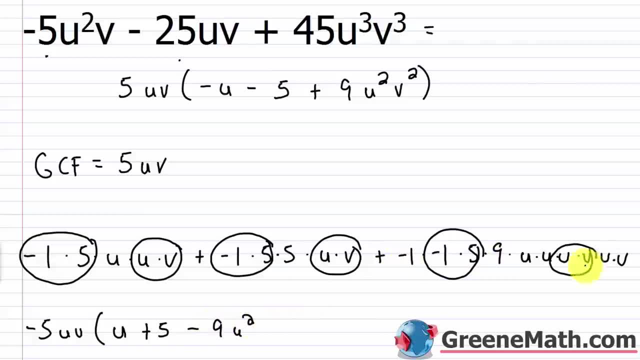 a negative: 9- u squared, v squared. Okay, So, using this little trick, I can do it the other way, And you can see that all I did was change the sign of everything. Instead of this being negative, it's positive. Instead of this being negative, it's positive. 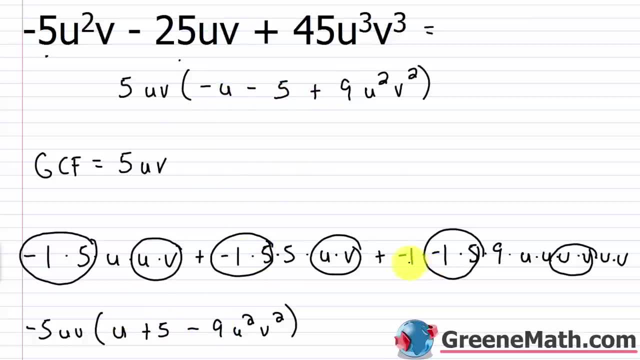 Instead of this being positive, it's negative. So you can always use little tricks like negative 1 times negative. 1 is positive 1 to kind of write this in a longer format. I know some of you like to write it this way, versus dividing each term. I've seen a lot of students. 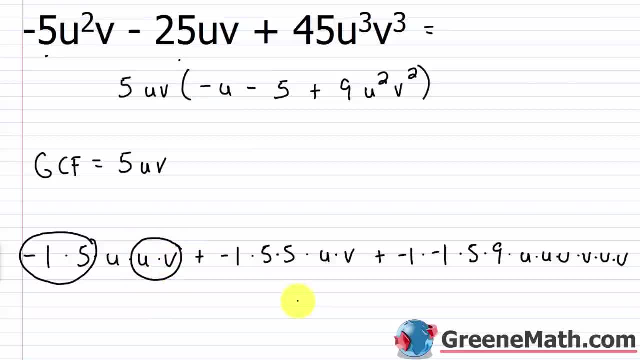 And then for the variable part, it's uv. So I'm going to circle that in each case. 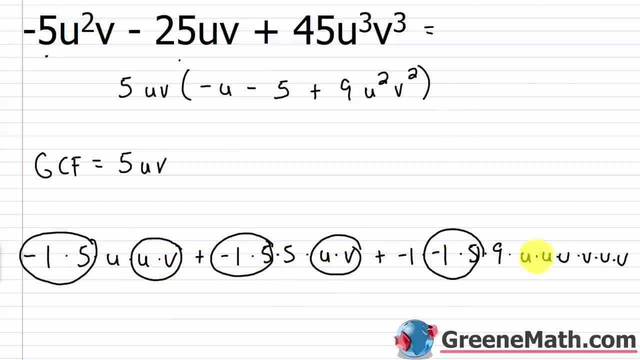 Negative 5uv. So negative 5. And then uv. 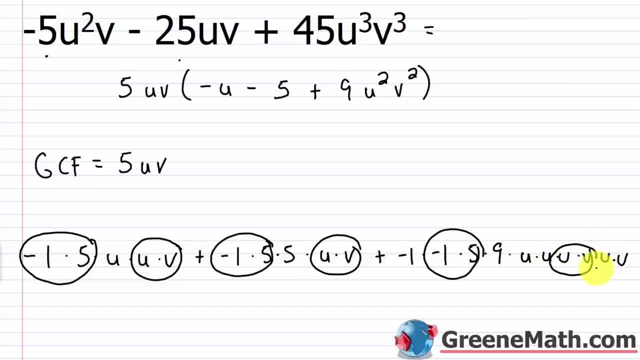 So if you think about it here, what would be left? If I pulled out the negative of the GCF? Well, if I pulled out a negative 5uv, what's left in this case? I would have a u only. 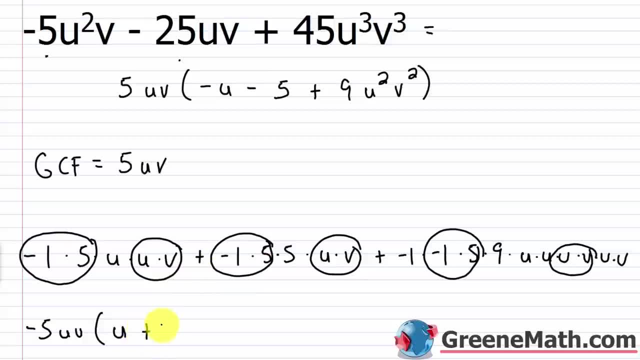 And then here I would have a plus 5. 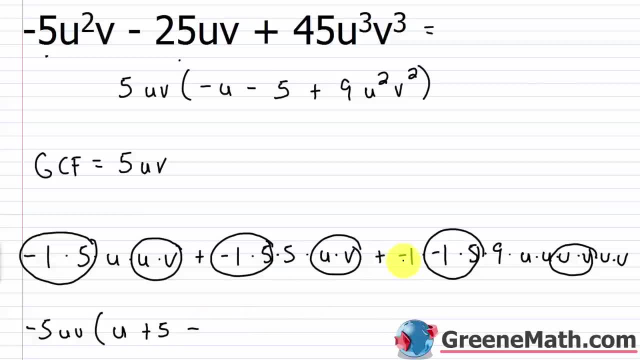 Then here I would have a negative, a negative 9u squared v squared. Okay. 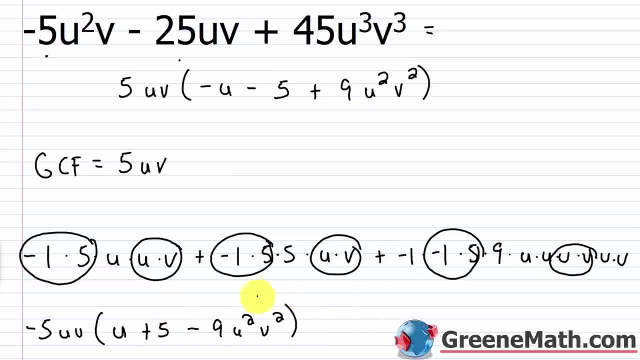 So using this little trick, I can do it the other way. And you can see that all I did was change the sign of everything. Instead of this being negative, it's positive. Instead of this being negative, it's positive. Instead of this being positive, it's negative. 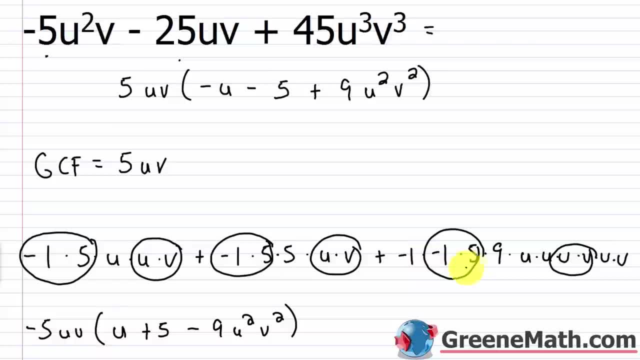 So you can always use little tricks like negative 1 times negative 1 is positive 1 to kind of write this in a longer format. I know some of you like to write it this way 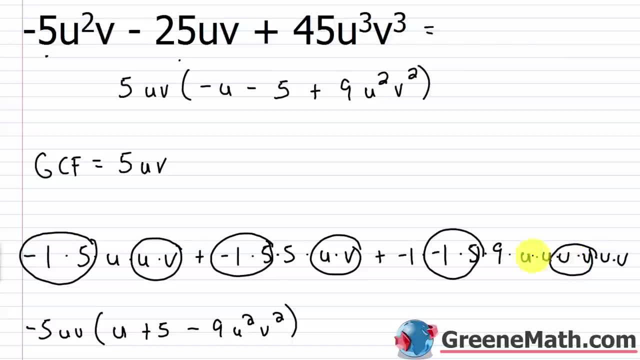 versus dividing each term. I've seen a lot of students have a lot of success with this and just really hate doing the division. So if this works for you, I think that's great. 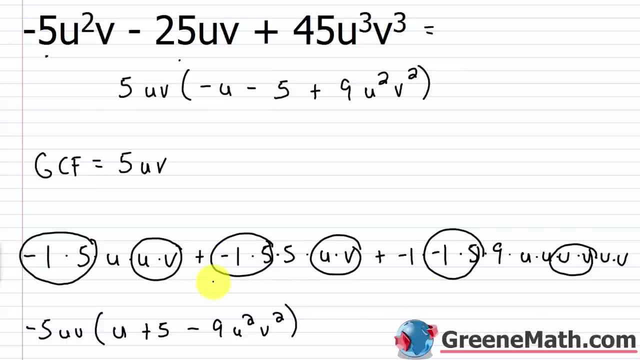 Use it. If it doesn't, then by all means, you know, use the division. Either way, you get the right answer. All right. Let's take a look at the final problem here. 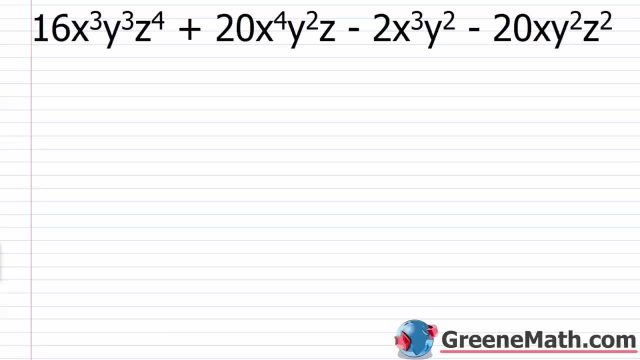 I have 16x cubed y cubed z to the fourth plus 20x to the fourth y squared z minus 2x cubed y squared minus 20xy squared z squared. All right. 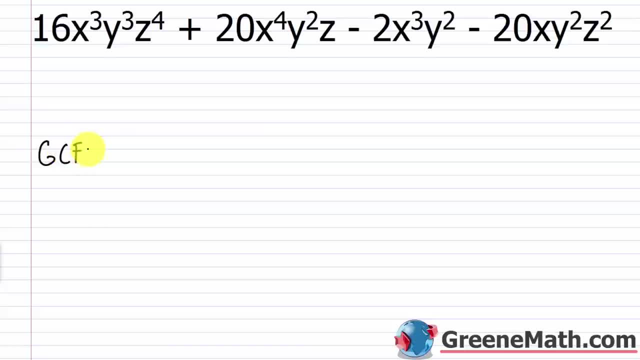 So what is the GCF? Well, for the number part, I know it's going to be a 2. Right? Because everything is divisible by 2. 2 is the smallest number, so it's going to be a 2. For the variable part, everything has an x. 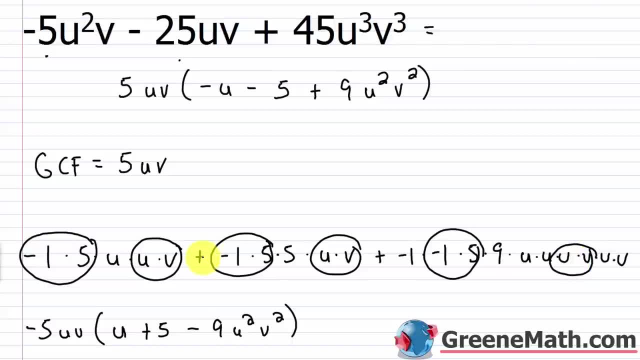 have a lot of success with this and just really hate doing the division. So if this works for you, I think that's great. Use it. If it doesn't, then by all means, you know, use the division. Either way, you get the right answer. 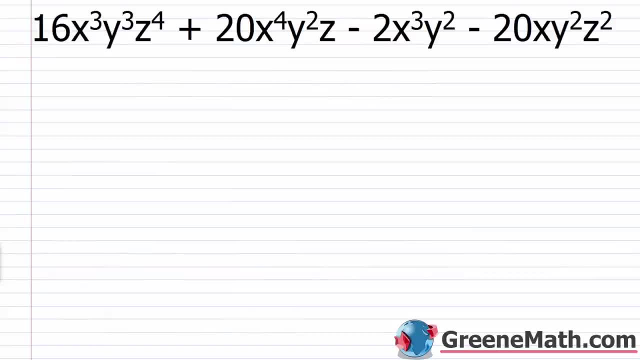 Alright, let's take a look at the final problem. here I have 16 x cubed y, cubed z to the fourth, plus 20 x to the fourth, y squared z minus 2 x cubed y squared. minus 20 x y squared z squared. Alright. 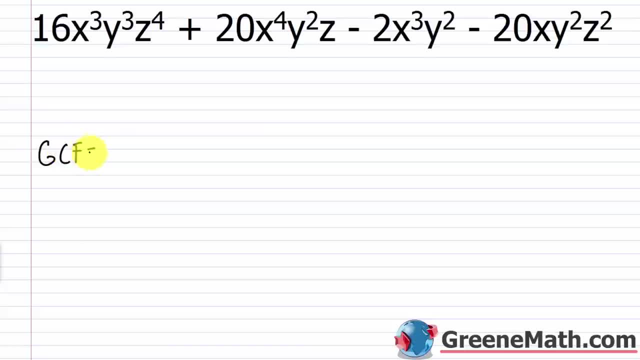 so what is the GCF? Well, for the number part, I know it's going to be a 2.. Right, because everything's divisible by 2.. 2 is the smallest number, so it's going to be a 2.. For the variable part, everything has an x. 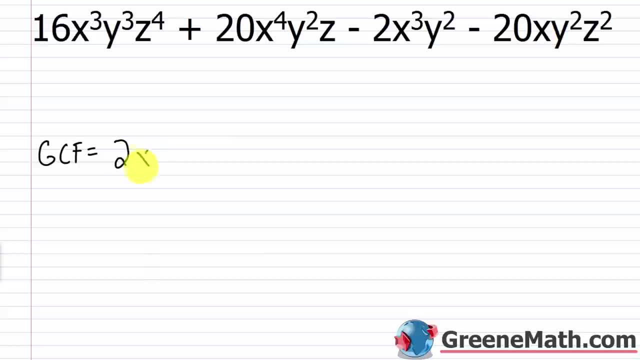 the smallest exponent is a 1.. Then everything has a y, The smallest exponent is a 2. But not everything has a z. This doesn't have a z here, So the GCF would be 2 x, y squared. Now pull this. 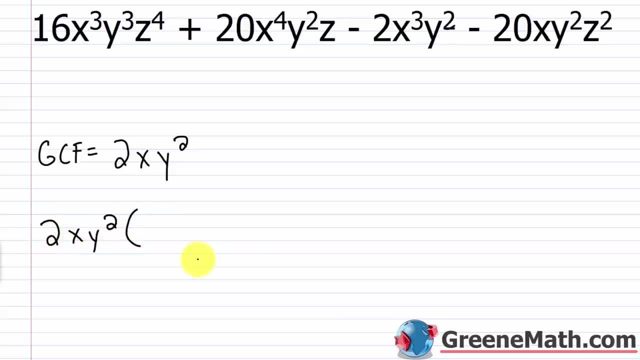 out and we're going to have 4 terms here. So if I divide this by 2 x y squared, So 16 x cubed y cubed z to the fourth over 2 x y squared, And eventually you're going to be able to do this in your head. But for right now I want to 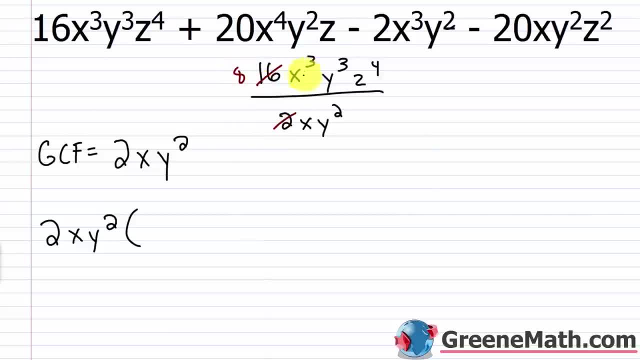 just make it completely clear: 16 over 2 is 8.. x cubed over x is x squared, y cubed over y squared is y. So this is going to give me 8 x squared y, z to the fourth, And then we'll have plus. 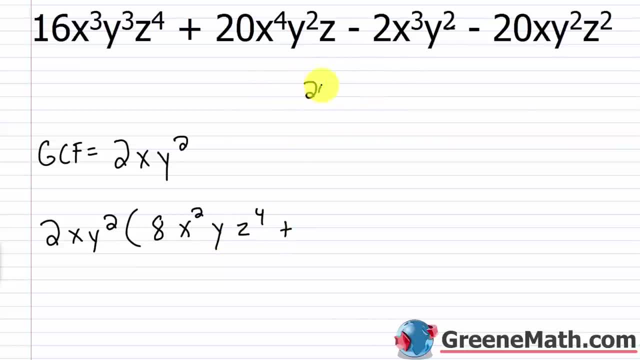 for the next term I'm going to have 20 x to the fourth power, y squared, z over again, 2, x, y squared. So 20 over 2 is 10.. x to the fourth over x is x cubed, y squared over y squared is 1.. 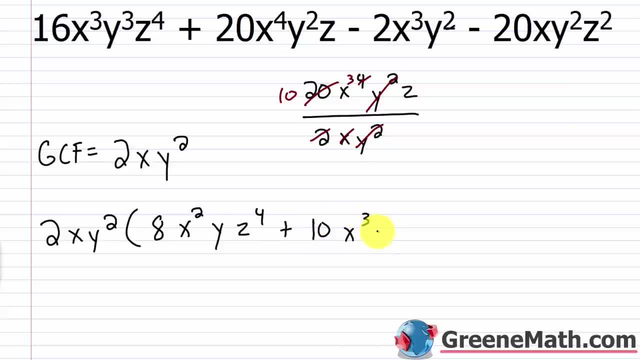 So I'm going to have 10 x cubed z and then move on to the next term. I have minus 2 x cubed y squared And this is over again. the GCF of 2 x y squared, So negative 2 over 2, is 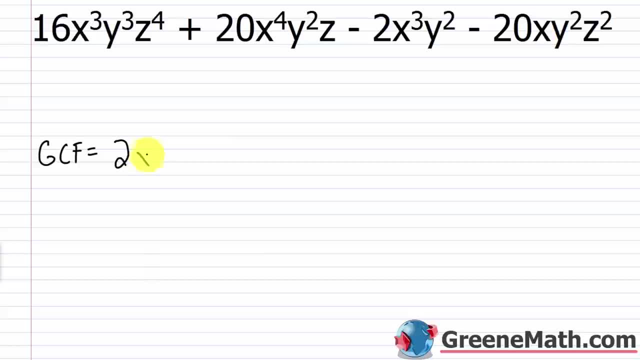 The smallest exponent is a 1. Then everything has a y. The smallest exponent is a 2. But not everything has a z. This doesn't have a z here. 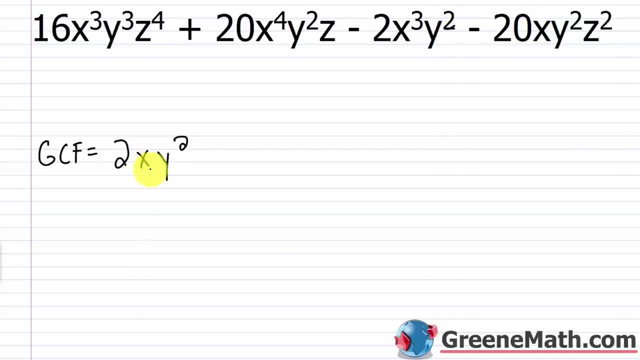 So the GCF would be 2xy squared. Now, pull this out. 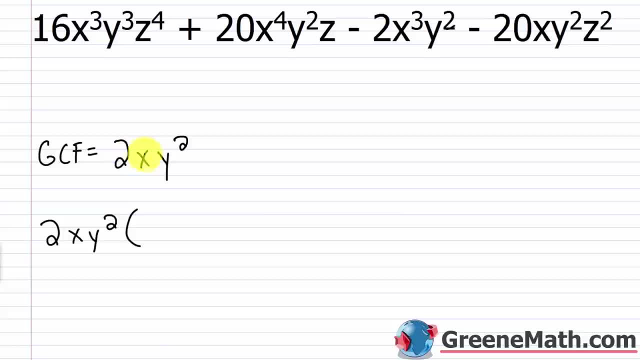 And we're going to have four terms here. So if I divide this by 2xy squared, 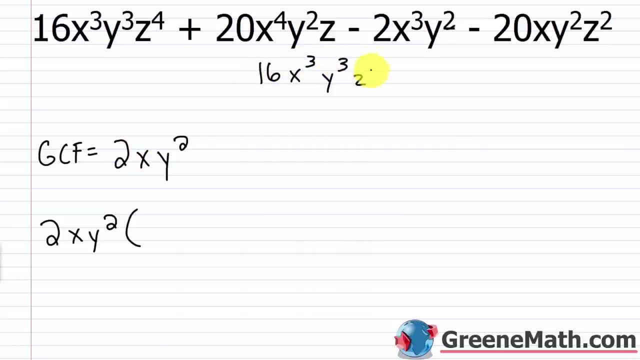 so 16x cubed y cubed z to the fourth over 2xy squared. 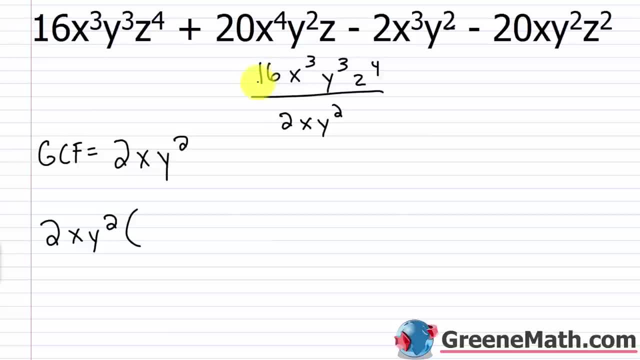 And eventually, you're going to be able to do this in your head. But for right now, I want to just make it completely clear. 16 over 2 is 8. x cubed over x is x squared. y cubed over y squared is y. 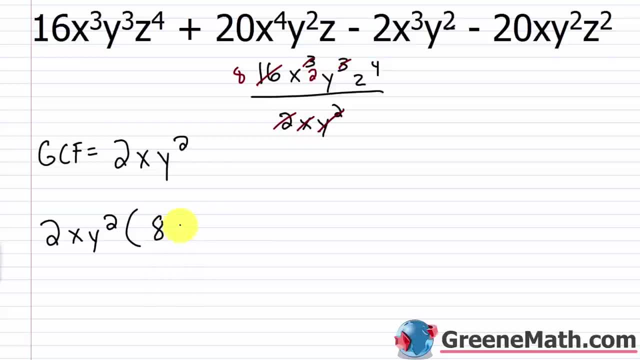 So this is going to give me 8x squared yz to the fourth. And then we'll have plus. For the next term, I'm going to have 20x to the fourth power y squared z 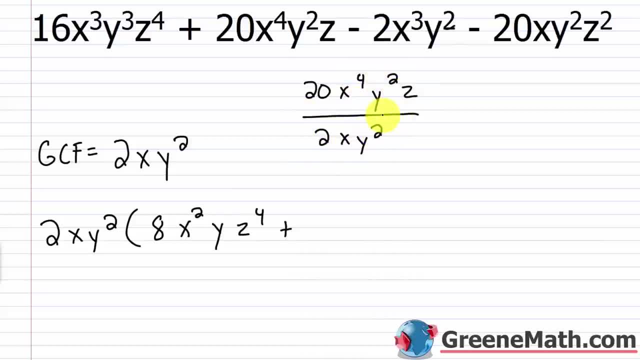 over, again, 2xy squared. So 20 over 2 is 10. x to the fourth over x is x cubed. 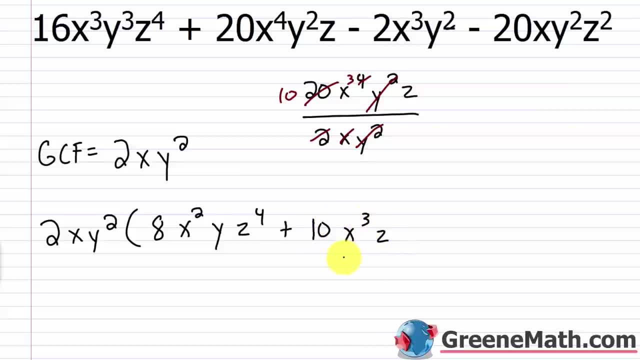 So I'm going to have 10x cubed z. 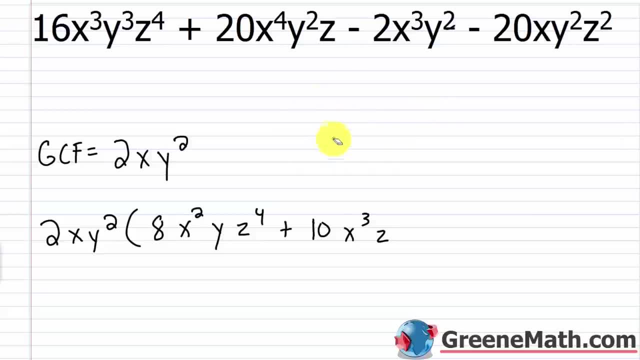 And then move on to the next term. 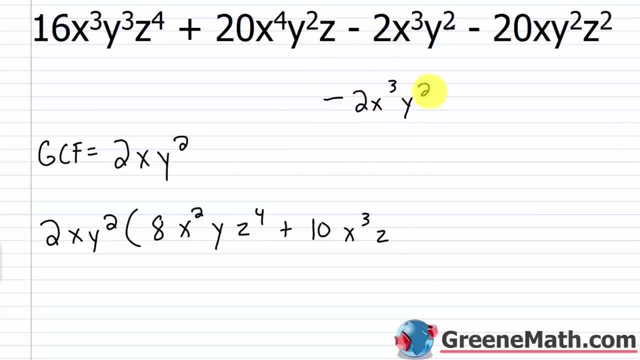 I have minus 2x cubed y squared. 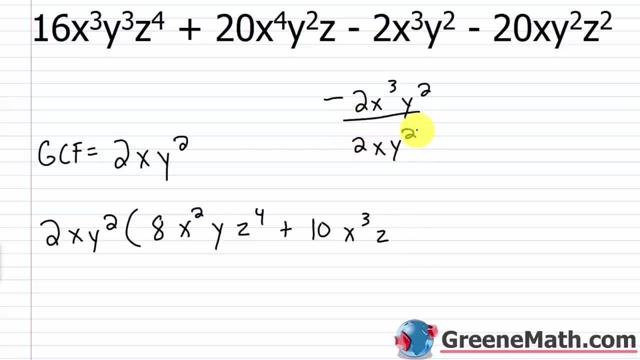 And this is over, again, the GCF of 2xy squared. So negative 2 over 2 is negative 1. x cubed over x is x squared. 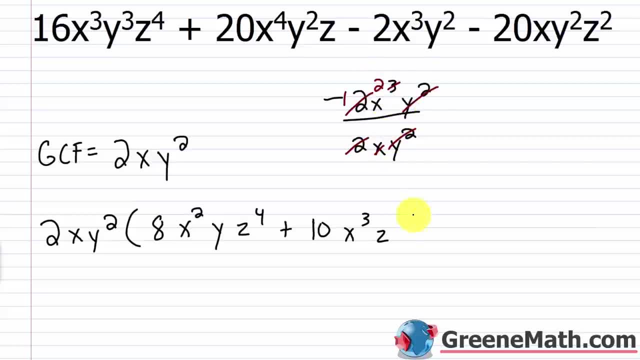 y squared over y squared is 1. So this would be negative x squared. And then lastly, we have this term here, which is negative 20xy squared. 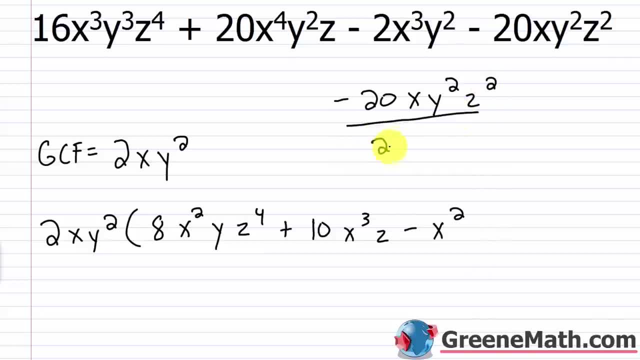 y squared z squared over 2xy squared. OK. 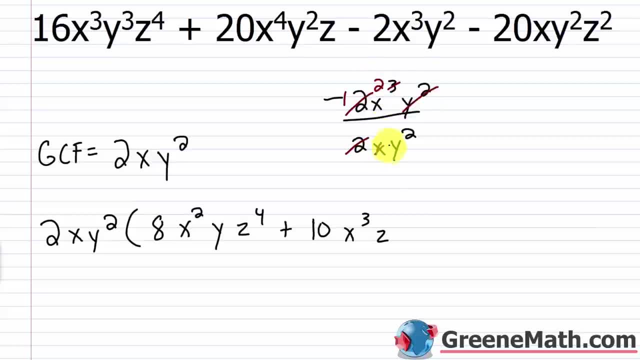 negative: 1.. x cubed over x is x squared. y squared over y squared is 1.. So this would be negative x squared. And then, lastly, we have this term here which is negative 20: x. y squared. z squared over 2 x. 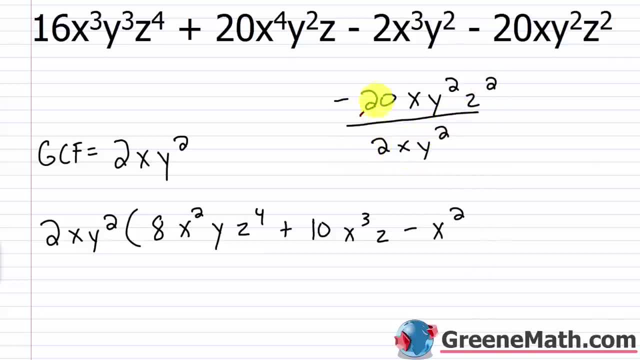 y squared. So let's divide this by this and I'll get negative 10.. And then x over x is 1.. y squared over y squared is 1.. So essentially I'll just have negative 10 z squared, So minus 10. 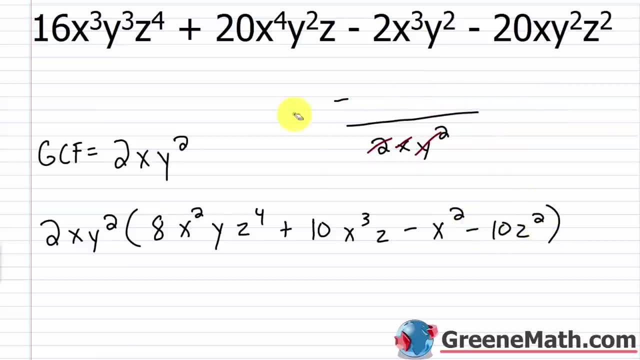 z squared. So now I'm done, So let's erase this here And let me kind of put equals And let me move this down Over here And I'll move this up. Okay, So we've written this as 2. 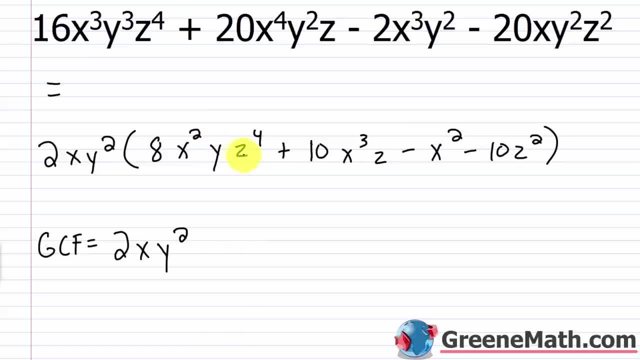 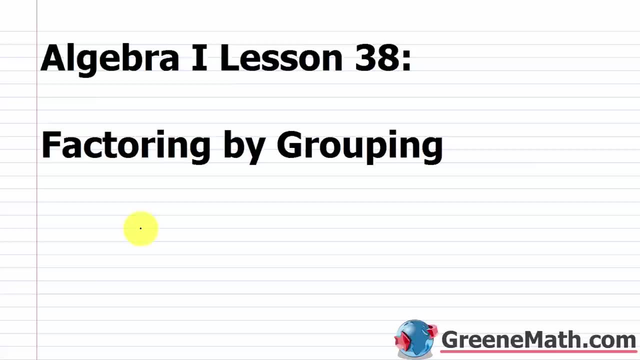 x- y squared times the quantity 8 x squared, y z to the fourth, plus 10 x cubed. z minus x squared. minus 10 z squared. Hello and welcome to Algebra 1, Lesson 38.. In this video we're going to learn about factoring. 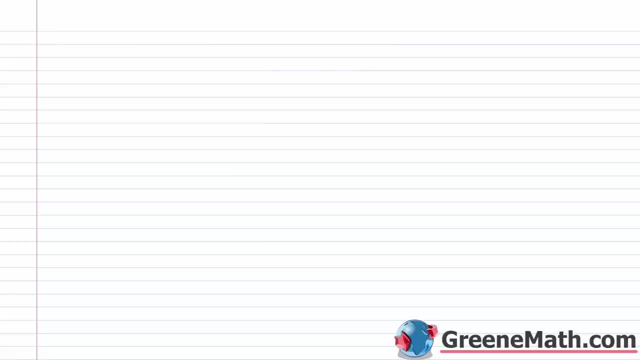 by grouping. So before we kind of jump in and start talking about factoring by grouping, I just want to revisit what we did in the last lesson. So our last lesson, as you'll recall, was all about factoring out the GCF, or again, the greatest common. 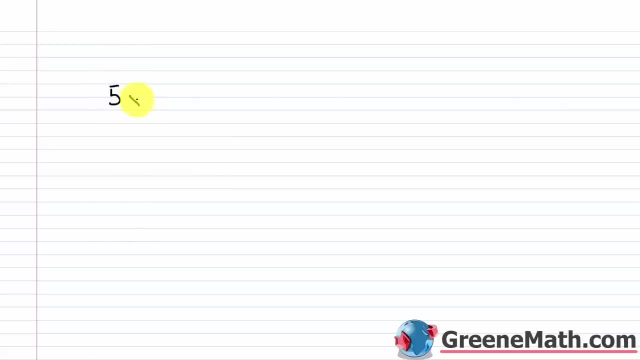 factor. So if I had something like, let's say, 5 x to the fifth power minus 15 x cubed, How would I go about factoring out the GCF? Well, essentially, the first thing I'd have to do is find the GCF. So between these two terms, 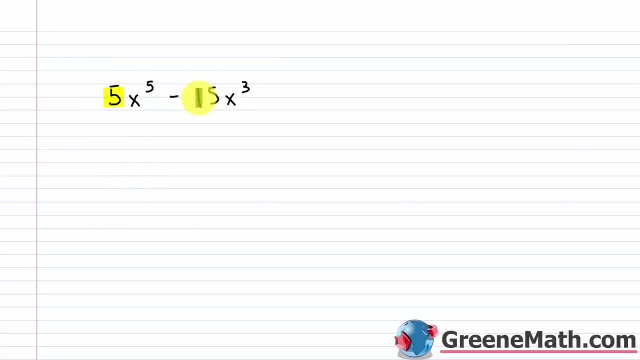 I have a 5 here and I have a 15 here. Now, 15 is the divisible by 5, right, 15 divided by 5 is 3.. So the number part for the GCF would be a 5.. That's simple. 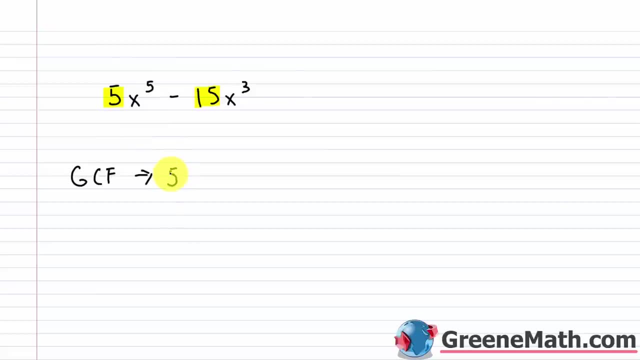 enough Now for the variable part. it's even simpler. In each case I have an x and I just go with the smallest exponent that appears in either term. So the smallest exponent is a 3. so this would be 5 x cubed for the GCF. So let's divide this by this. And I'll get negative 10. 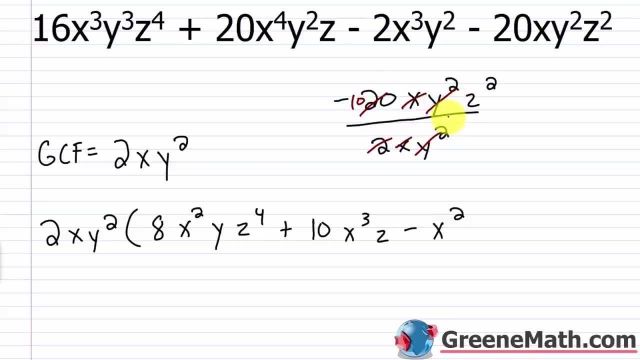 And then x over x is 1. y squared over y squared is 1. 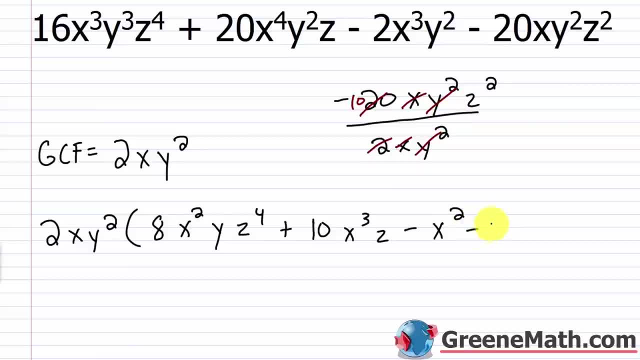 So essentially, I'll just have negative 10z squared. So minus 10z squared. 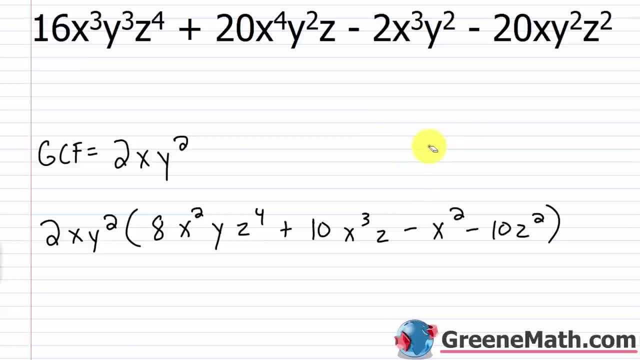 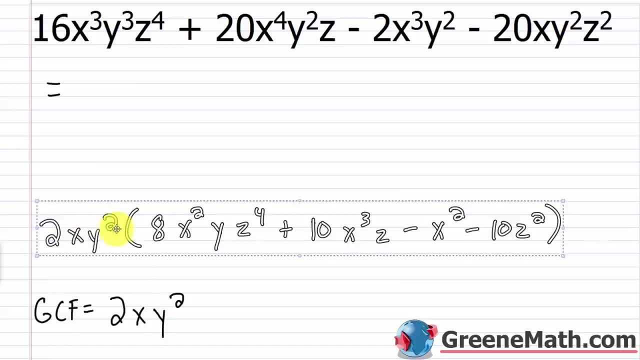 So now I'm done. So let's erase this here. And let me kind of put equals. And let me move this down over here. I'll move this up. OK. 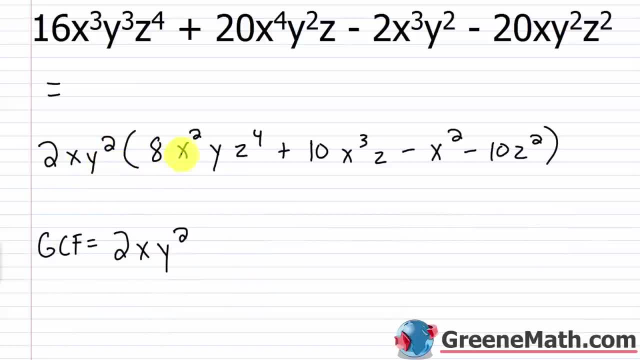 So we've written this as 2xy squared times the quantity 8x squared yz to the fourth 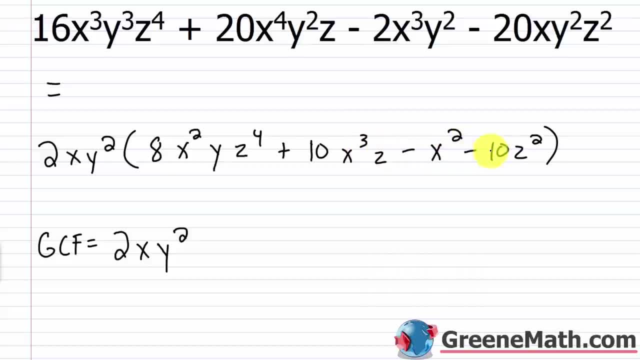 plus 10x cubed z minus x squared minus 10z squared. 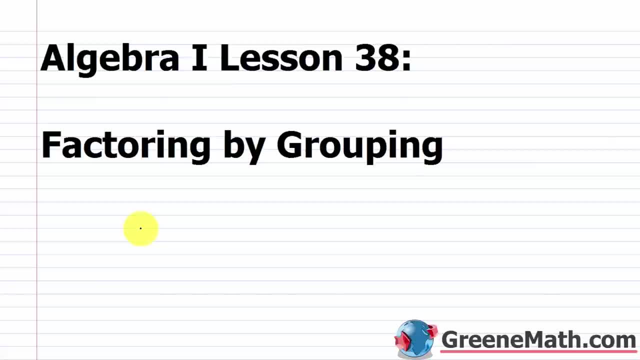 Hello, and welcome to Algebra 1 Lesson 38. In this video, 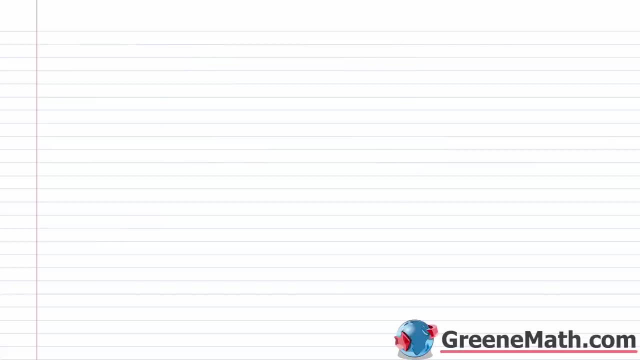 we're going to learn about factoring by grouping. So before we kind of jump in and start talking about factoring by grouping, I just want to revisit what we did in the last lesson. 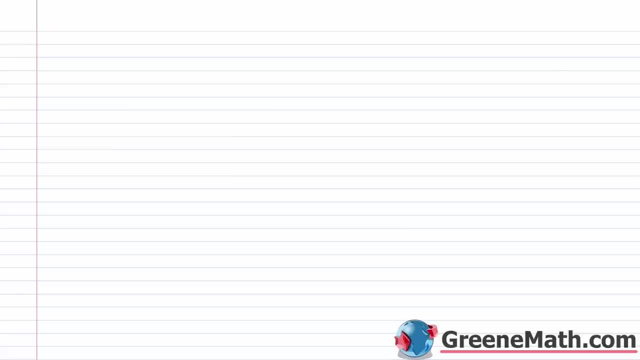 So our last lesson, as you'll recall, was all about factoring out the GCF, or again, the greatest common factor. So if I had something like, let's say, 5x to the fifth power minus 15x cubed, how would I go about factoring out the GCF? Well, essentially, the first thing I'd have to do is find the GCF. So between these two terms, I have a 5 here, and I have a 15 here. 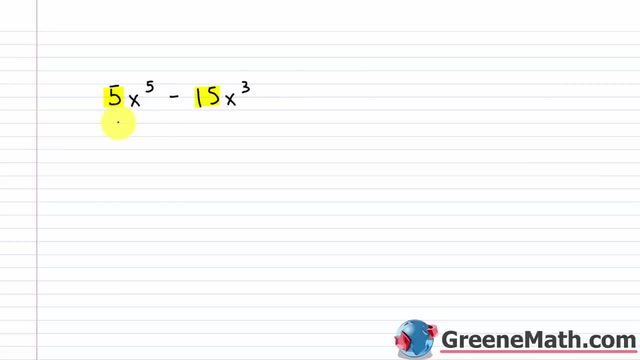 Now, 15 is divisible by 5, right? 15 divided by 5 is 3. 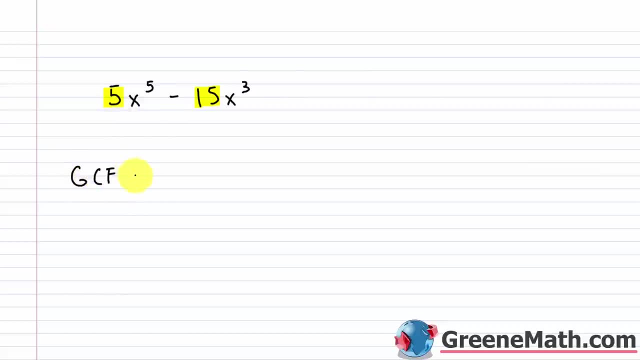 So the number part for the GCF would be a 5. That's simple enough. 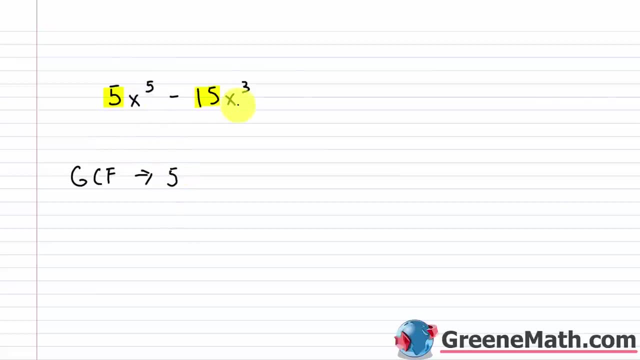 Now, for the variable part, it's even simpler. In each case, I have an x, 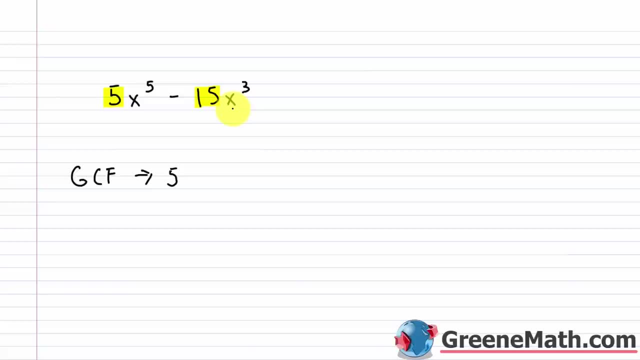 and I just go with the smallest exponent that appears in either term. So the smallest exponent is a 3, so this would be 5x cubed for the GCF. 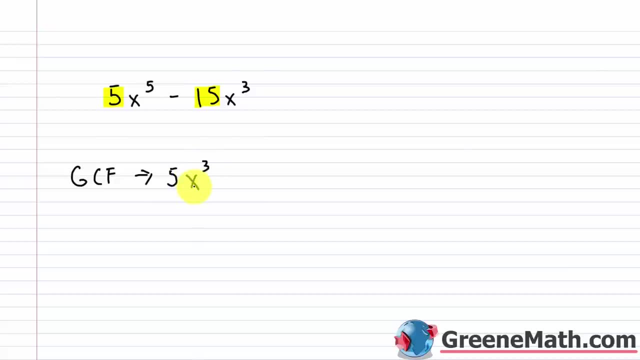 Now, that's the easy part. Once we've gathered our GCF, what we're going to do, we're going to put equals, and we're going to place that GCF outside of a set of parentheses. 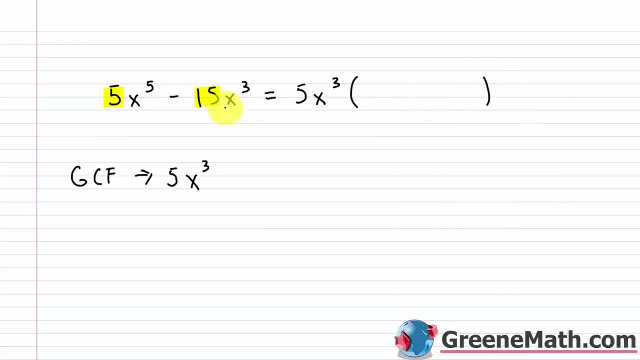 Now, what's going to go inside the parentheses? We'll have two spaces for those two terms, and then our minus sign. Don't forget about that. 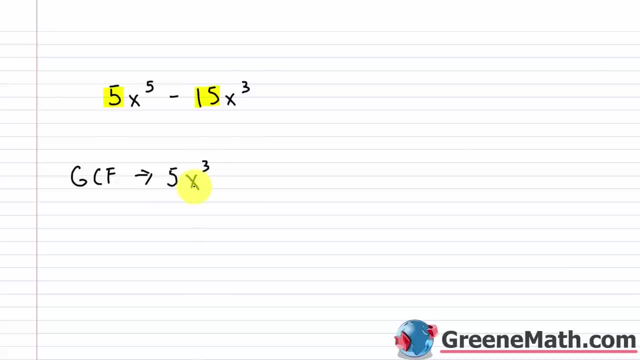 Now, that's the easy part. Once we've gathered our GCF, what we're going to do is we're going to put equals and we're going to place that GCF outside of a set of parentheses. Now, what's going to go inside? 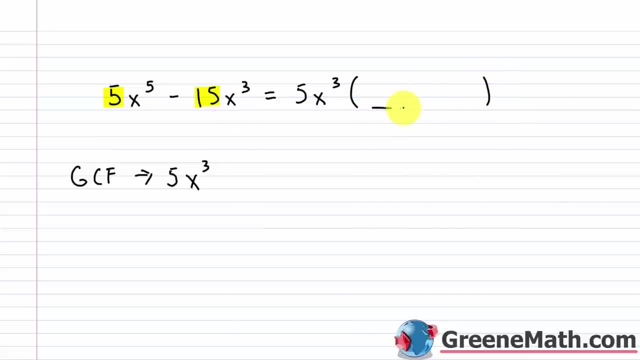 the parentheses. We'll have two spaces for those two terms and then our minus sign. Don't forget about that. Now, how do I figure out what goes in each space? Well, I want you to think for a minute about what you're doing. 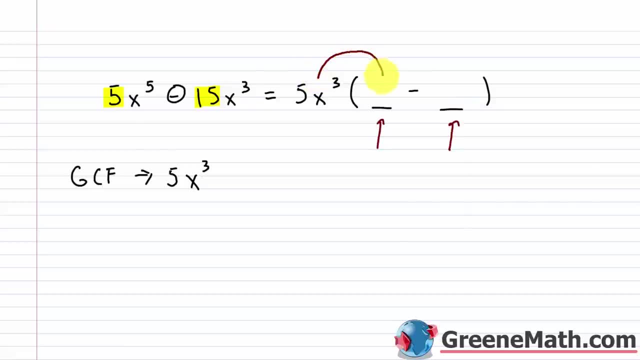 We talked about this in the lesson. This is going to be multiplied by this and it's going to give me this, So we have multiple multiplication here. The opposite of multiplication is division. So if I want to figure out what this unknown is here, all I need to do is take 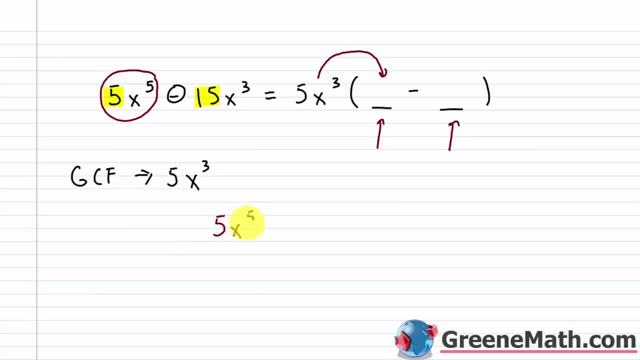 the original term, which is 5 x to the fifth power, and divide it by this 5 x cubed, and I will get my missing term here. So 5 over 5 is 1. that would cancel. and then x to the fifth power over x cubed is x squared. 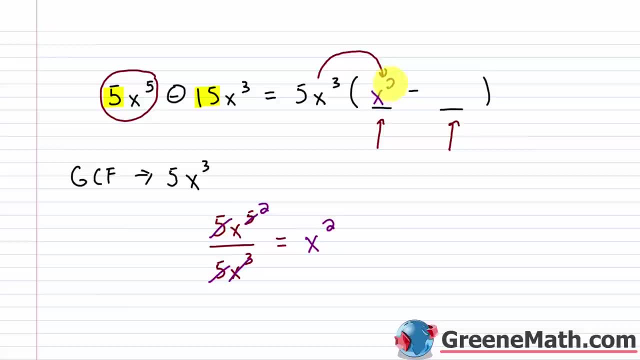 So this would be x squared here, And you can see that works itself out, because 5 x cubed times x squared would get me back to the original 5 x to the fifth power. We're going to do the same thing for this term, right here. 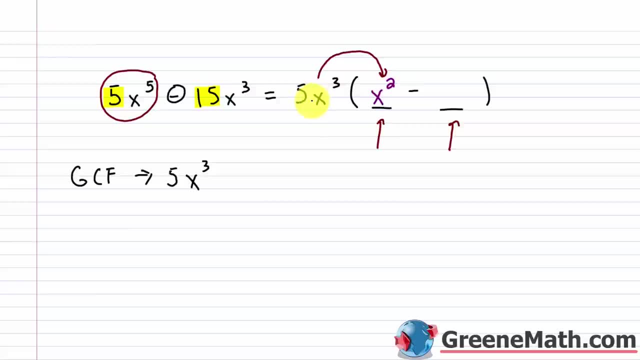 This 15 x cubed, I'm going to again divide it by the GCF, So 15 x cubed over 5 x cubed, because again this times this will give me back this. So again I can find that unknown by dividing this. 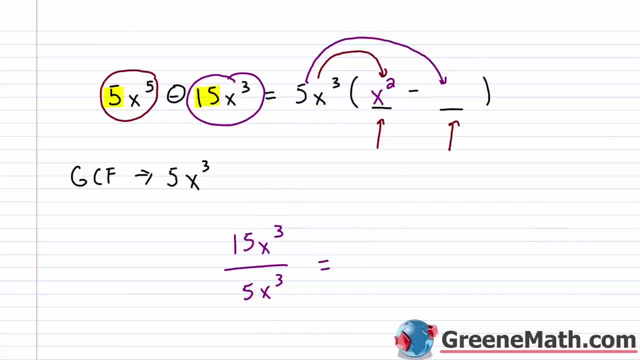 by this. So now what we're going to do? I'm going to cancel the 15 with the 5. this is going to be a 3, and then x cubed over x cubed is 1.. So this would just be a 3 here. 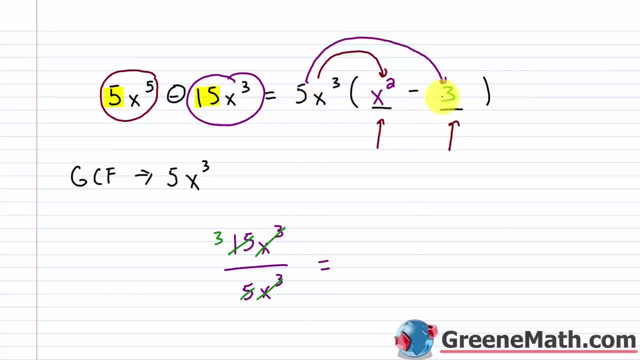 And again, check that with multiplication 5 x cubed times 3 gives me 15 x cubed. So if you went back, if you went back and you used your distributive property, 5 x cubed times x squared would give you 5 x to the fifth power. 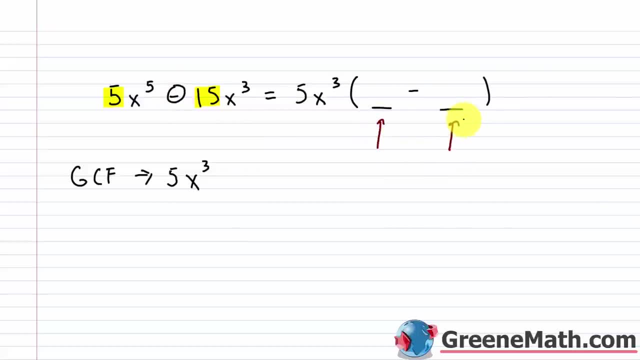 Now, how do I figure out what goes in each space? Well, I want you to think for a minute about what you're doing. 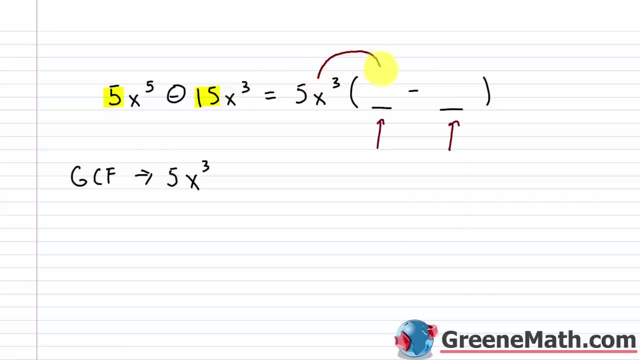 We talked about this in the lesson. This is going to be multiplied by this, and it's going to give me this. So we have multiplication here. The opposite of multiplication is division. 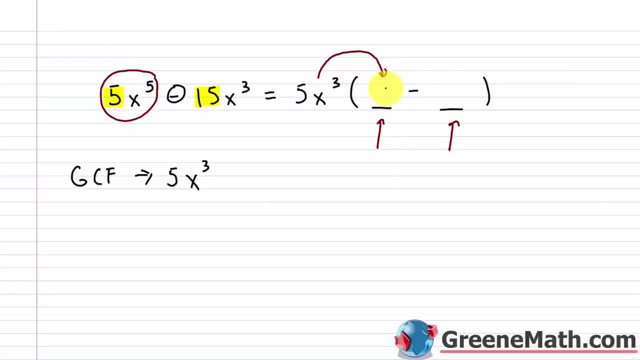 So if I want to figure out what this unknown is here, all I need to do is take the original term, which is 5x to the fifth power, and divide it by this 5x cubed, this 5x cubed, and I will get my missing term here. So 5 over 5 is 1. That would cancel. And then x to the fifth power over x cubed is x squared. 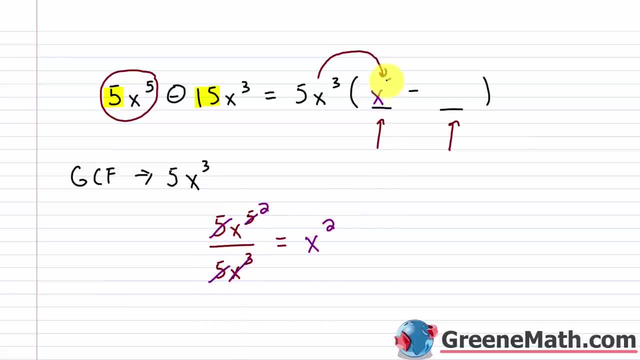 So this would be x squared here. And you can see that works itself out because 5x cubed times x squared would get me back to the original 5x to the fifth power. 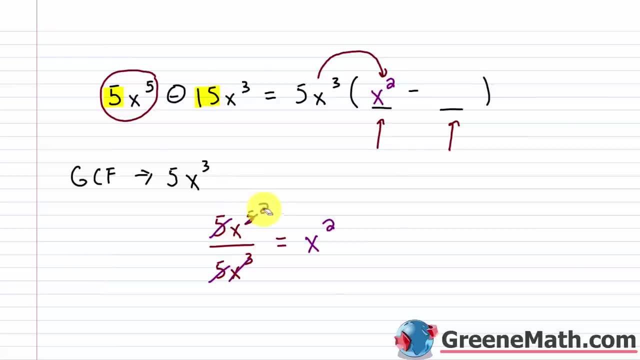 We're going to do the same thing for this term right here, this 15x cubed. I'm going to, again, divide it by the GCF, so 15x cubed over 5x cubed, because, again, this times this, okay, will give me back this. So, again, I can find that unknown 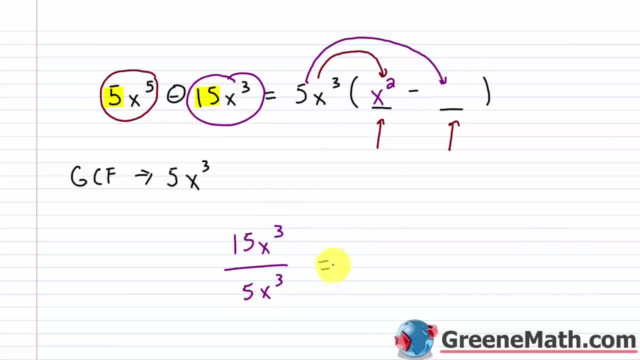 by dividing this by this. Okay, so now what we're going to do, I'm going to cancel the 15 with the 5. This is going to be a 3. And then x cubed over x cubed is 1. So this would just be a 3 here. And, again, check that with multiplication. 5x cubed times 3 gives me 15x cubed. 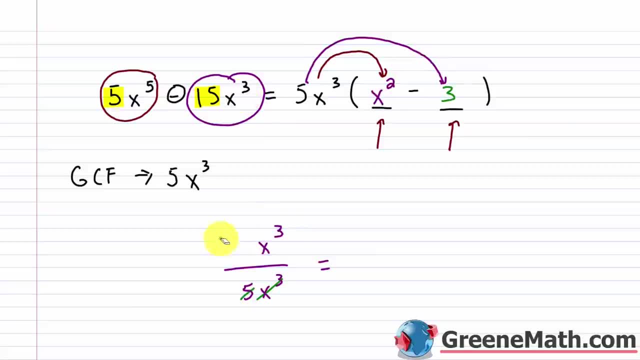 So if you went back, okay, if you went back and you used your distributive property, 5x cubed times x squared, would give you 5x to the fifth power. Then minus, you have a minus there. 5x cubed times 3 would give you 15x cubed. So you get back what you started with. And, again, one more time for those of you who don't like to do the division. 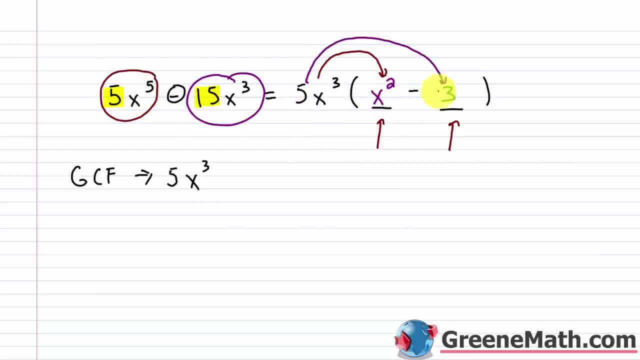 Then minus. you have a minus there. 5 x cubed times 3 would give you 15 x cubed. So you get back what you started with. And again one more time for those of you who don't like to do the division: 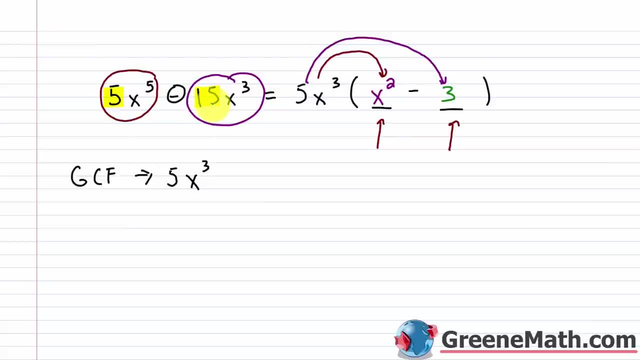 I know it's confusing for some of you. you could write this out if you wanted to. You could say: this is 5 times. let's say we do it like this: x cubed times x squared minus. we could do 5 times 3 times x cubed. 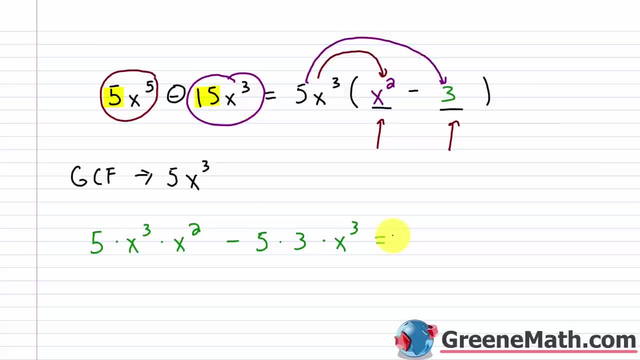 Now, if I'm going to pull out a 5 x cubed, so let me kind of use a different color here. I'm going to pull this out here and I've got to circle it here and here you just look at what would be left. so if I write a 5 x cubed here, 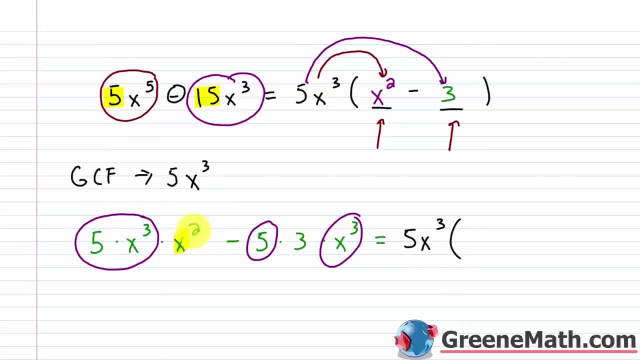 what would go in the space in each case is what's left. So you'd have an x squared there, so an x squared, then you've got your minus, and then what's left over here? Well, just a 3.. So that's an alternative method. 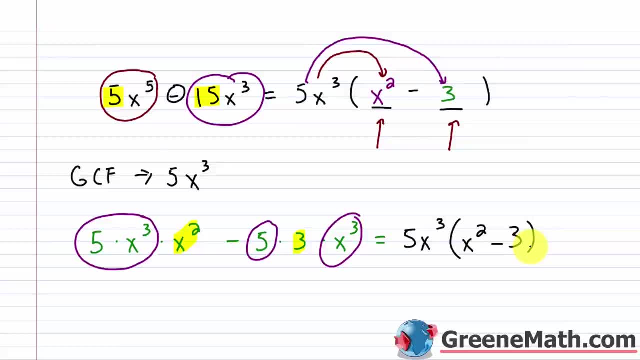 for those of you who don't like to do the division. I know it confuses some of you, especially in your Algebra 1. Once you get to Algebra 2, you've done this enough, so it'll kind of make more sense for you. but this is an alternative method. 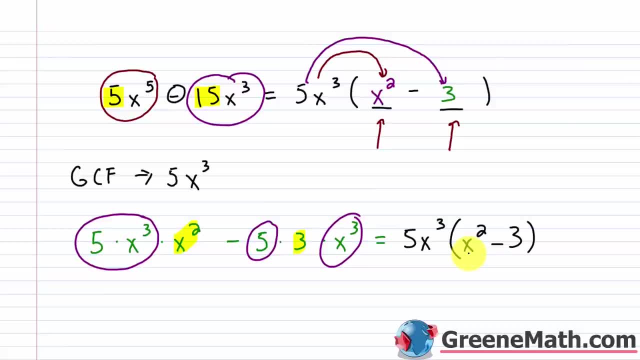 if you just can't get the division down. Okay, so let's look at something else. real quick, We're going to keep this, we're going to go to a different screen here and I want to show you something that's very similar to that, but just a little bit more complicated. 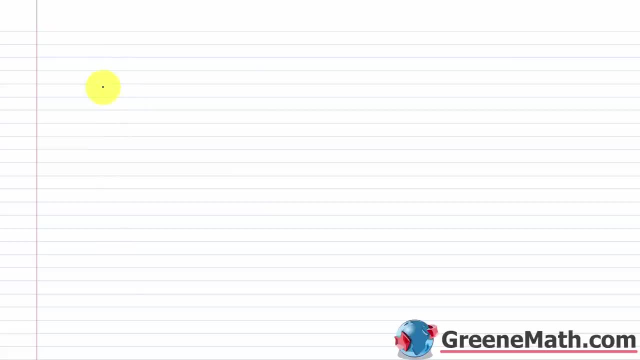 just kind of one step up the ladder. so let's say I saw something like x squared times 2 x minus 5, and then I had plus. let's say I had 3 x times 2 x minus 5. so at this point in your 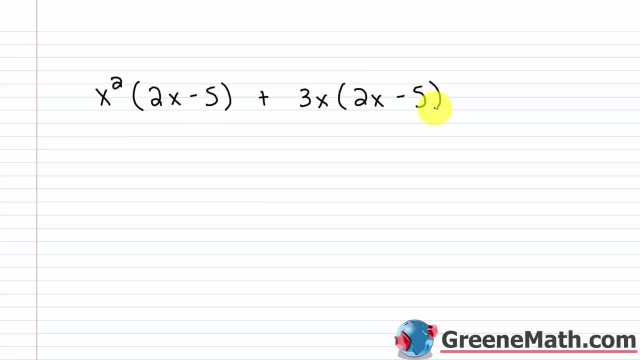 Algebra class. you've probably never seen or heard anybody talk about a common binomial factor, but that's what we have here. What I want to point your attention to is that this is multiplication. here, If you stick something outside of parentheses, you're multiplying. 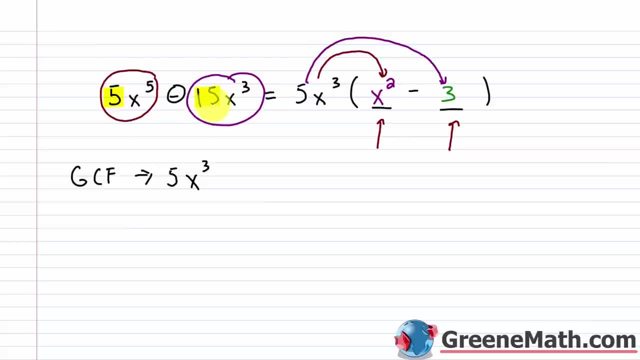 I know it's confusing for some of you. You could write this out if you wanted to. You could say, okay, this is 5 times, let's say we do it like this, x cubed times x squared minus, we could do 5 times 3, times x cubed. Now, if I'm going to pull out a 5x cubed, so let me kind of use a different color here. 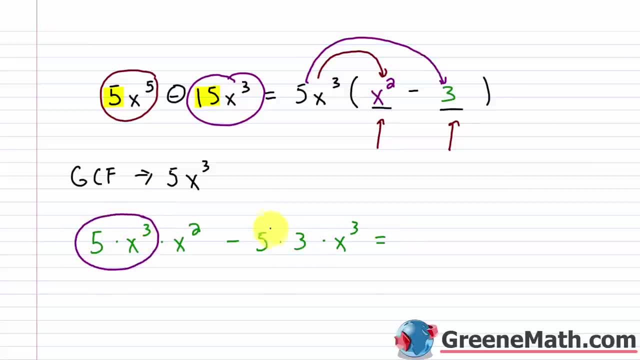 I'm going to pull this out here. And I've got to circle it here and here. You just look at what would be left. So if I write a 5x cubed here, what would go in the space in each case is what's left. So you'd have an x squared there. So an x squared. Then you've got your minus. And then what's left over here? Well, just a 3. 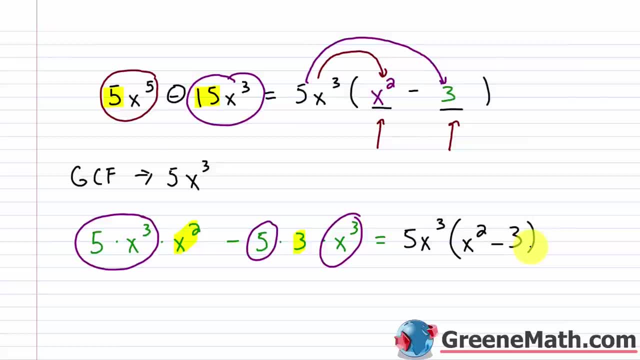 So just a 3 right there. So that's an alternative method for those of you who don't like to do the division. 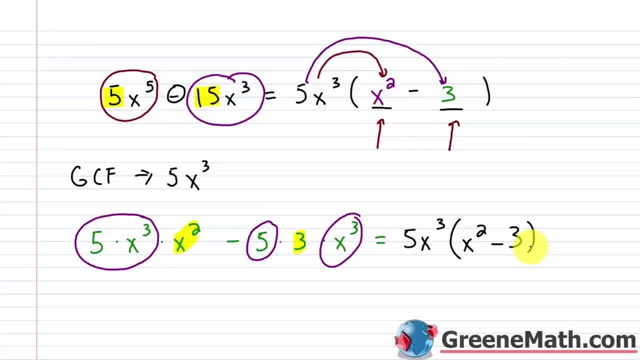 I know it confuses some of you, especially, you know, in your Algebra 1. 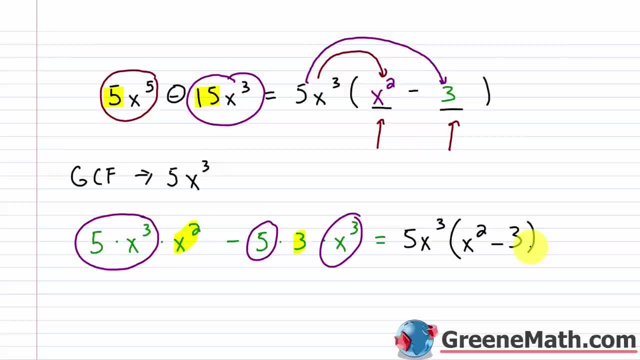 Once you get to Algebra 2, you've done this enough so it'll kind of make more sense for you. 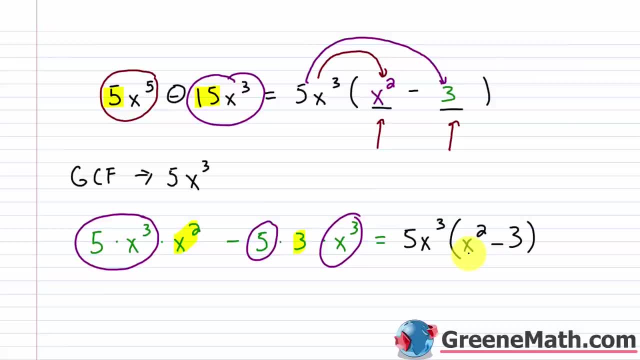 But this is an alternative method if you just can't get the division down. 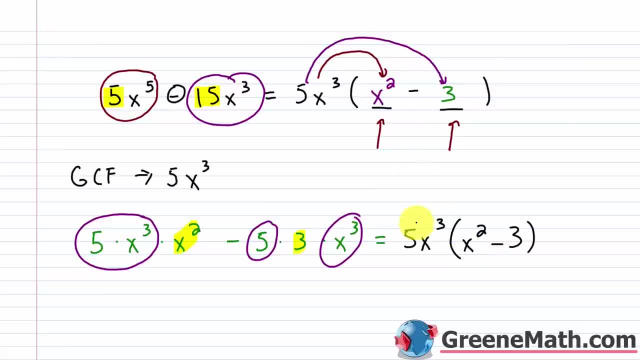 Okay, so let's look at something else real quick. We're going to kind of keep this. We're going to go to a different screen here. And I want to show you something that's very similar to that, 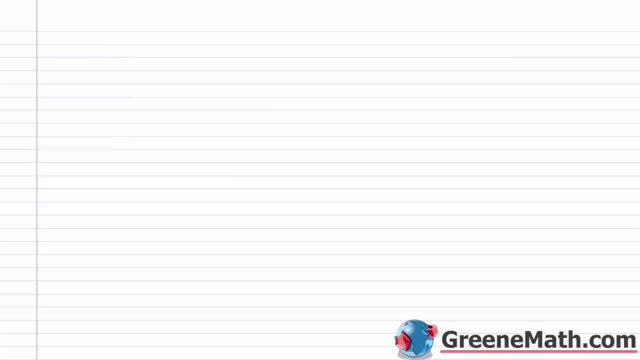 but just a little bit more complicated. Just kind of one step up the ladder. So let's say I saw something like 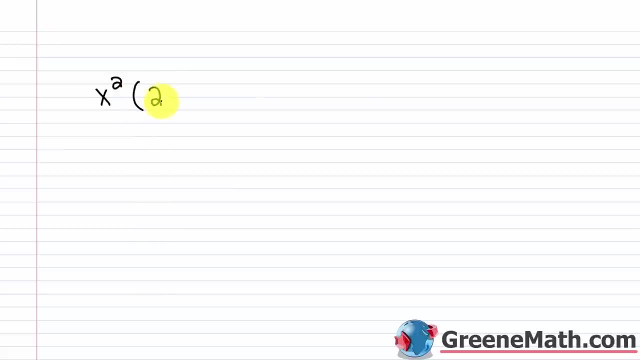 x squared times 2x minus 5. 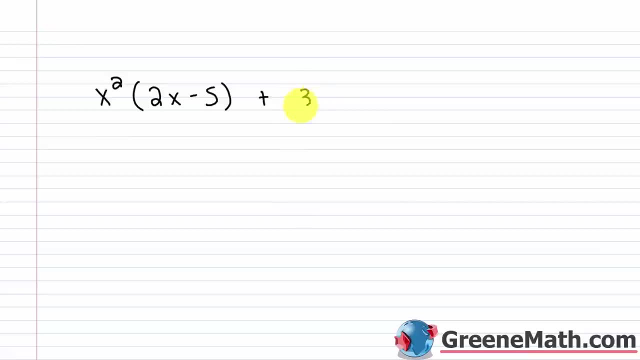 And then I had plus. Let's say I had 3x times 2x minus 5. 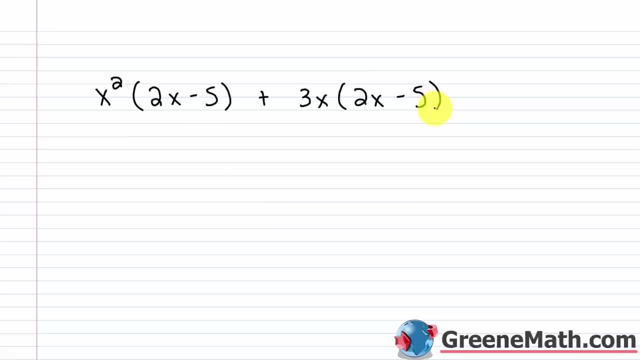 So at this point in your kind of Algebra class, you've probably never seen or heard anybody talk about a common binomial factor. But that's what we have here. The first thing I want to point your attention to is that this is multiplication here. Just take something outside of parentheses, you're multiplying. 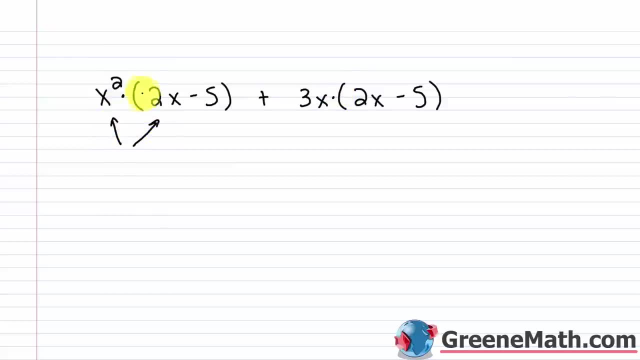 So I have x squared that is multiplying this whole quantity, 2x minus 5. So these are factors. Same thing goes over here. So I have 3 is a factor times x, which is a factor times, again, the quantity, 2x minus 5. So these are all factors. 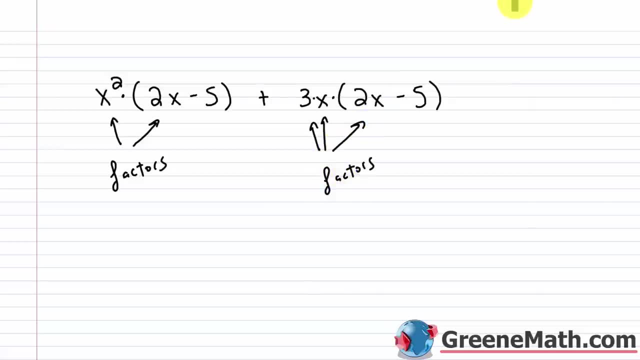 Now I have a common binomial factor, binomial is just a polynomial with two terms, of 2x minus 5 in each case. 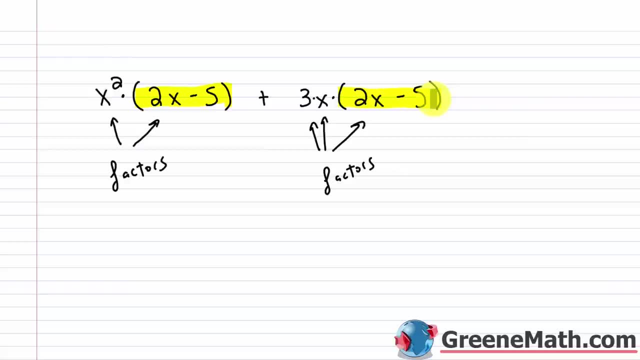 What I can do is I can actually factor that out the same way that I factored the 5x cubed out in this example here. So let me kind of show that to you. Let me erase this real quick. 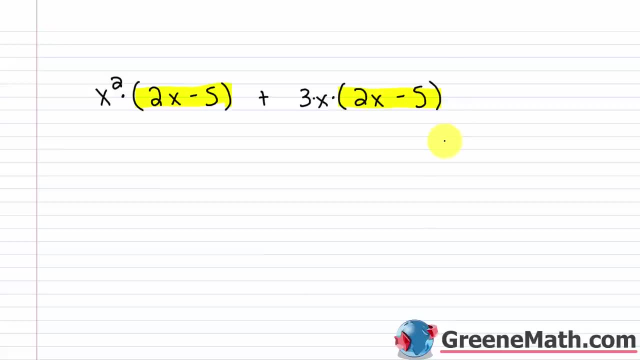 And I know it's a little confusing at first. So the first thing I'm going to do 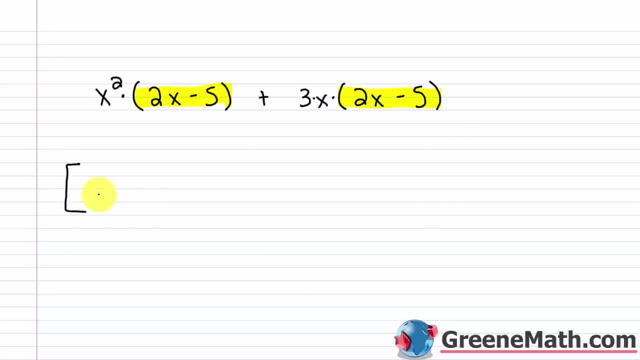 is put brackets around this just to make it obvious what I'm going to do. 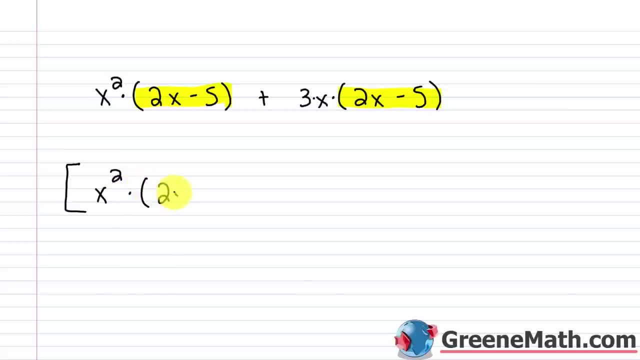 So x squared times, again, 2x minus 5 plus 3x times 2x minus 5. 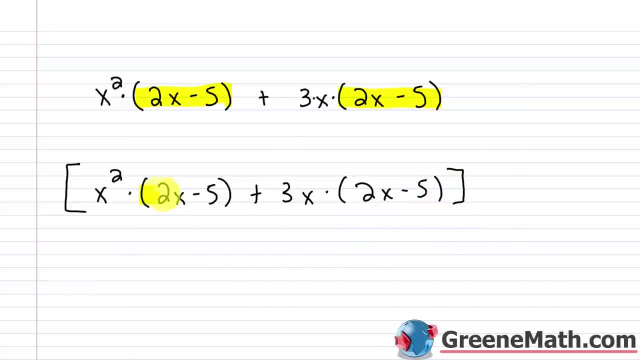 Now if I was to pull this out of the brackets, let me kind of scroll down, and I'm going to visually show that to you. 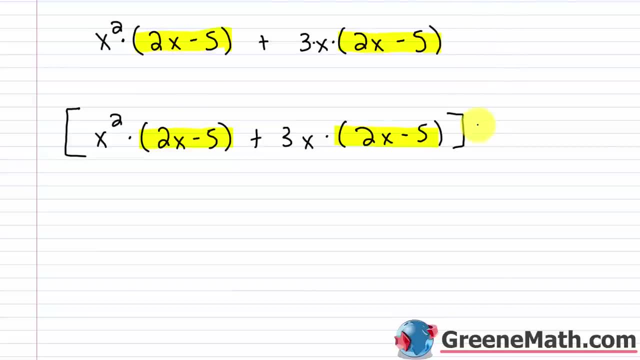 So let's say I drag this, down here, and I pull it out. So I'd have 2x minus 5 out in front of the brackets now. So let me put the brackets there. 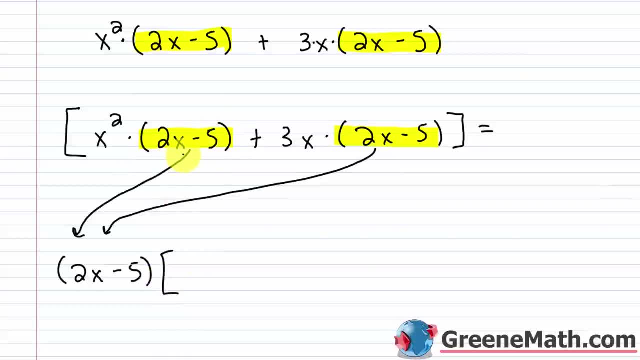 What's going to be left in each case? Well I've pulled this out from here, so it's not there. You can kind of think about it as we did in the last example with the division. 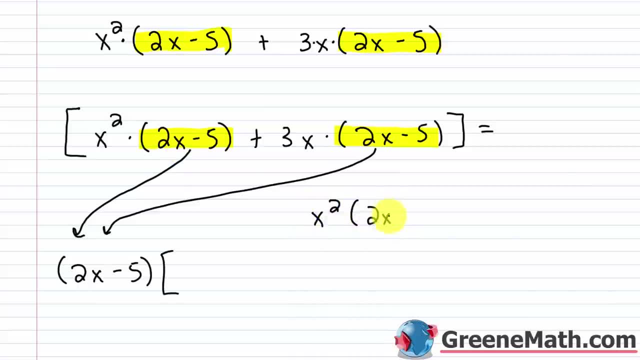 You could say if I had x squared times 2x minus 5, and this was over the quantity 2x minus 5, well I have a common factor here of 2x minus 5, so that would cancel, and I'm just left with x squared. 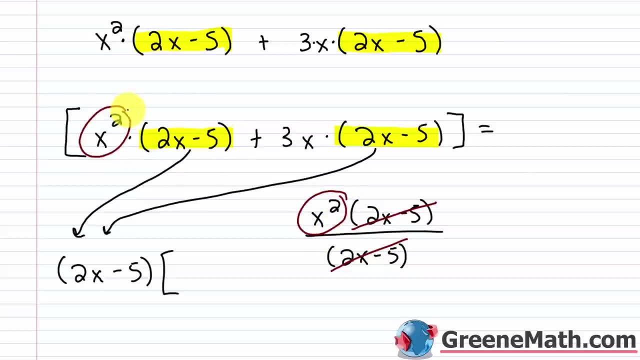 Again, you could just picture it as I'm pulling this out, so I'm just left with x squared. 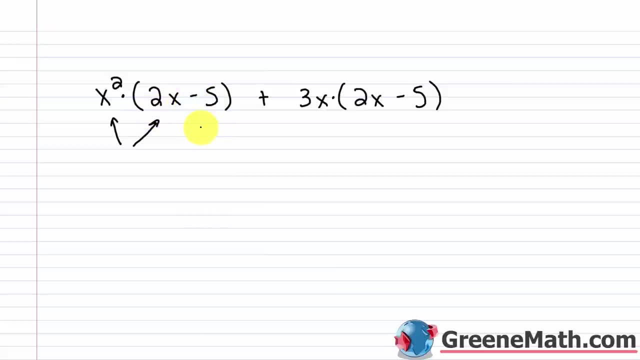 So I have x squared. that is multiplying this whole quantity 2 x minus 5. so these are factors. Same thing goes over here. so I have: 3 is a factor times x, which is a factor times again the quantity 2 x minus 5. 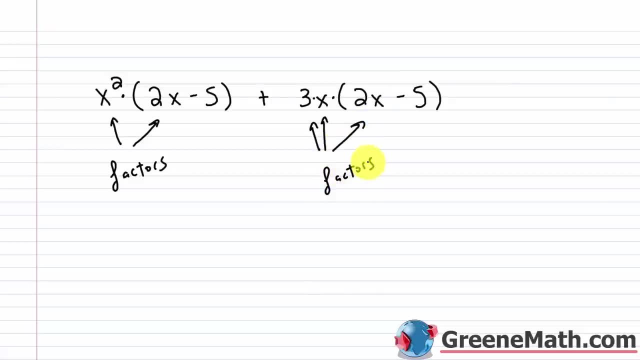 so these are all factors. Now I have a common binomial factor. binomial is just a polynomial with two terms of 2 x minus 5 in each case, what I can do is I can actually factor that out the same way that I factored. 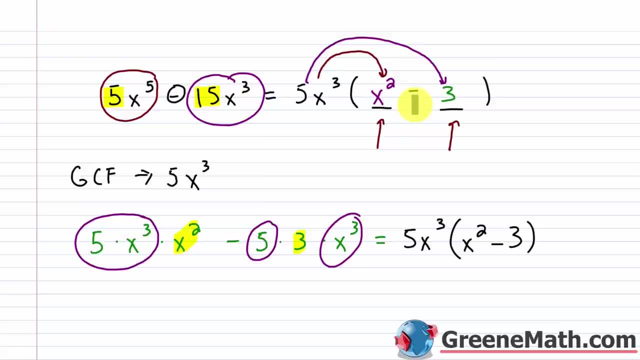 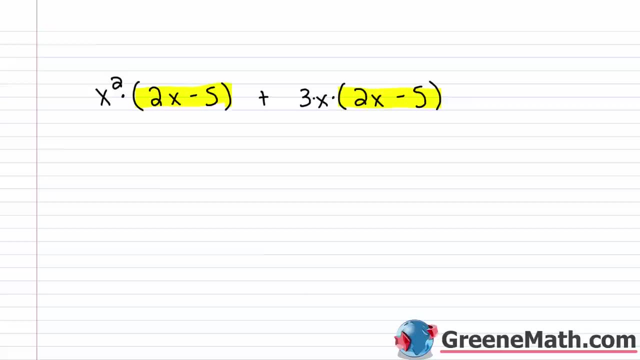 the 5 x cubed out in this example here. So let me kind of show that to you. let me erase this real quick, and I know it's a little confusing at first. so the first thing I'm going to do is put brackets around this. 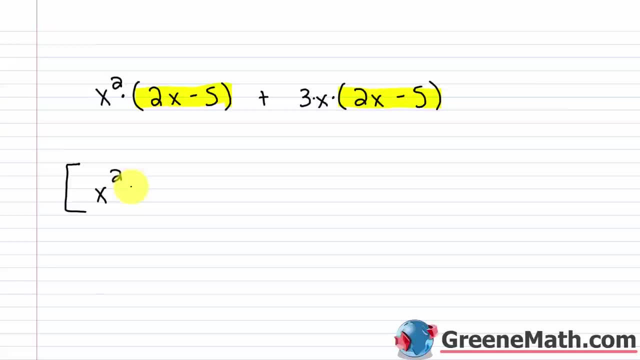 just to make it obvious what I'm going to do. so x squared times again 2 x minus 5, plus 3 x times 2 x minus 5. now, if I was to pull this out of the brackets, let me kind of scroll down and I'm going to visually show that to you. 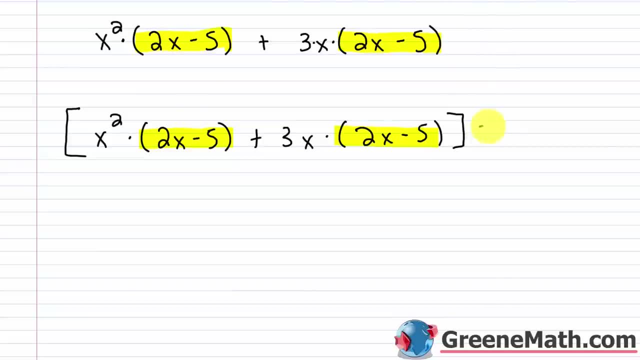 so let's say, I drag this down here and I pull it out 2 x minus 5 out in front of the brackets now. so let me put the brackets there. what's going to be left in each case? Well, I've pulled this out from here. 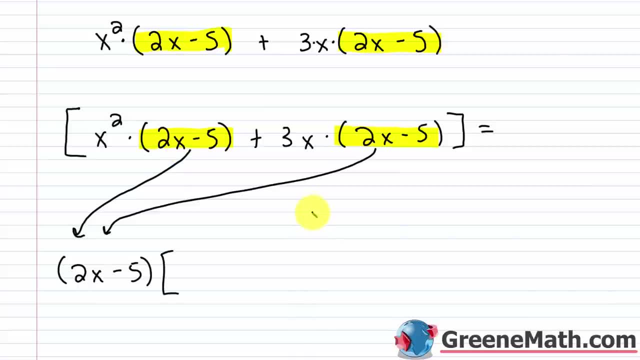 so it's not there. You can kind of think about it as we did in the last example with the division. you could say: if I had x squared times 2 x minus 5, and this was over the quantity 2 x minus 5, well, I have a common factor here. 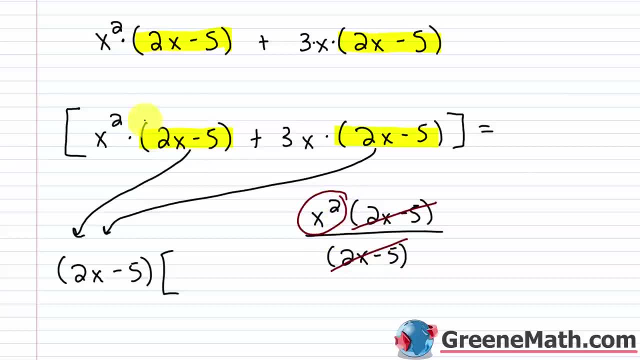 of 2 x minus 5, so that would cancel and I'm just left with x squared again. you could just picture it as I'm pulling this out of x squared. however, it makes sense for you. long story short, I'm just going to have x squared here. 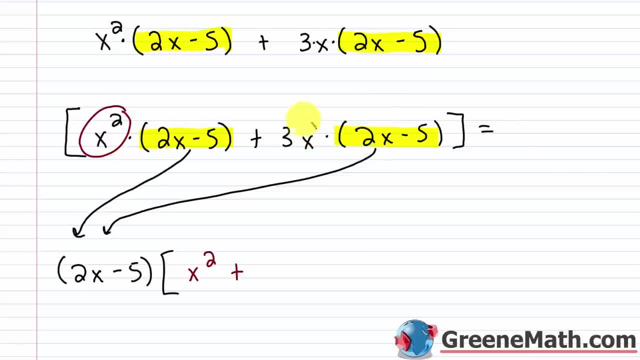 and then plus. this is pulled out from here, so I just have a 3 x, so plus 3 x, and instead of brackets I could just use parentheses- any grouping symbols will do- and what I have is I have 2 x minus 5 times I have x squared. 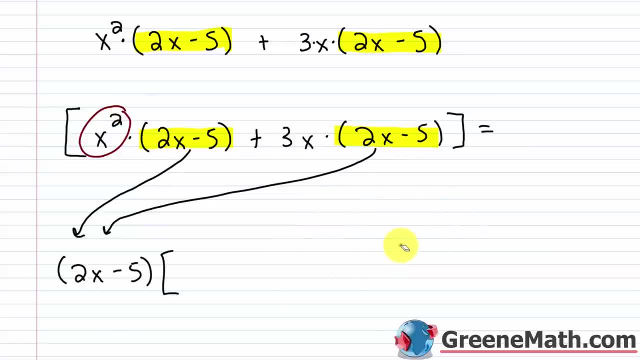 However it makes sense for you. Long story short, I'm just going to have x squared here, and then plus, this is pulled out from here, so I just have a 3x. So plus 3x, 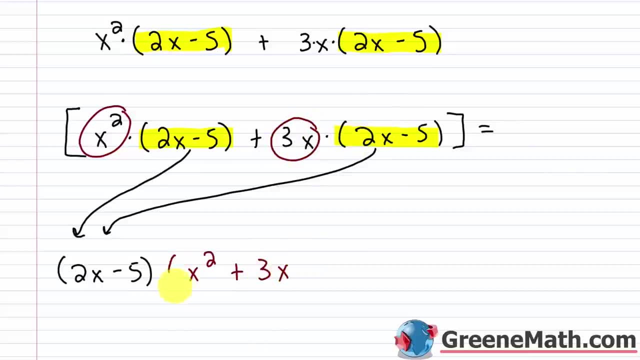 and instead of brackets, I could just use parentheses. Any grouping symbols will do. And what I have is, 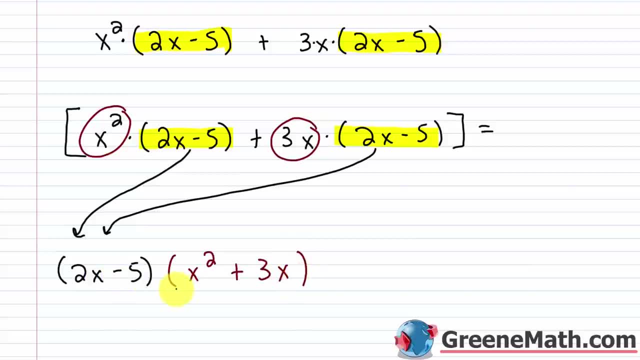 I have 2x minus 5 times, I have x squared plus 3x. Now we're going to learn later on that we can further factor this, and we can pull another x out, because that's common to each term here. But for right now, let's not even worry about that. 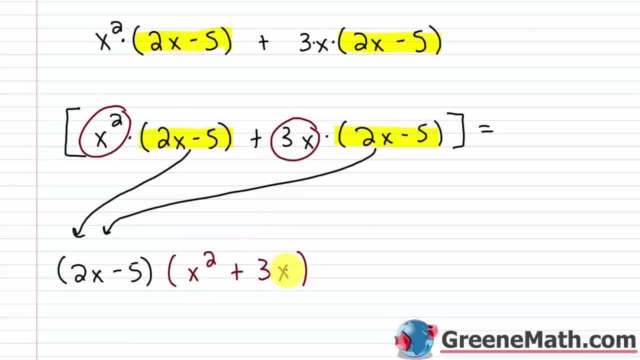 Let's just keep it as it is. So that is what factoring by grouping is going to entail. 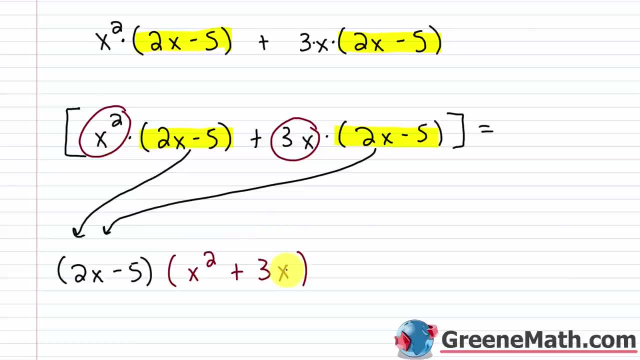 We're going to pull out a common binomial factor, and you're going to see that kind of moving forward. 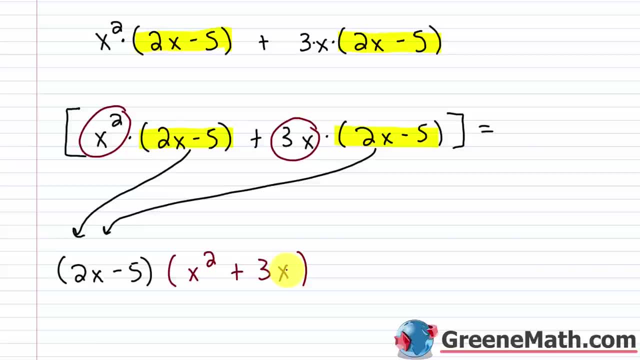 But before I go on, I want to show something to you. I want to prove to you that this is still equal to this. And a lot of you will doubt that. But I want you to notice, 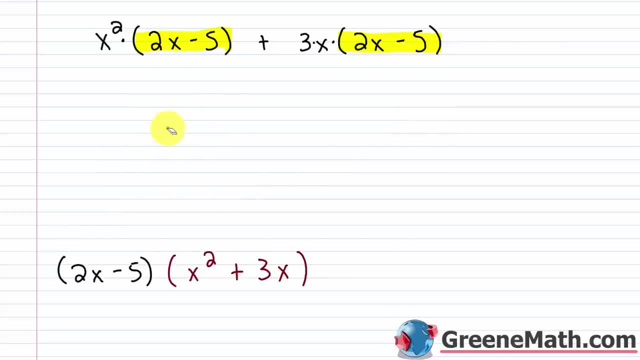 let me kind of erase this real fast. I want you to notice that this 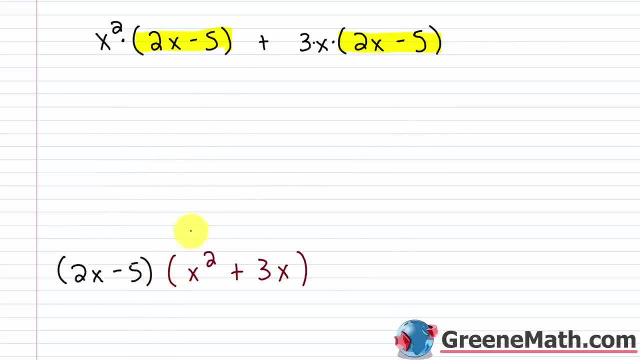 is nothing more than the way we used to multiply these guys together, right, before we learned FOIL. We would take this guy right here, and we'd multiply it by each term of the second polynomial. 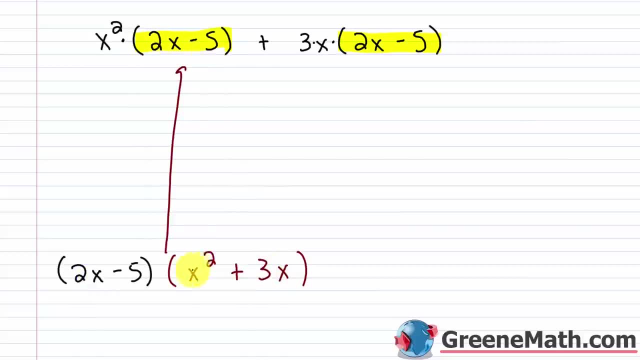 So that quantity 2x minus 5 would get multiplied by x squared, which it is here. Then plus, we'd have 3x multiplied by that polynomial here. 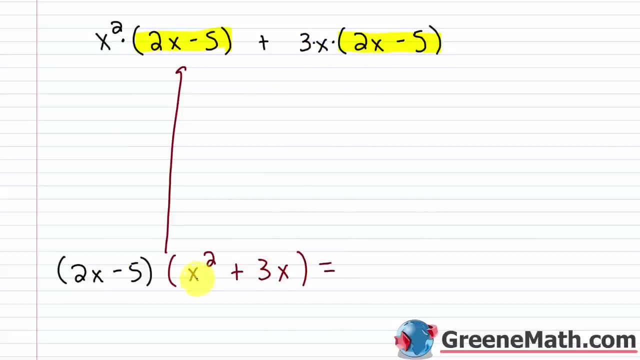 We'd multiply that polynomial again. So if I did FOIL on this, 2x times x squared is 2x cubed. The outer would be what? Plus 6x squared. 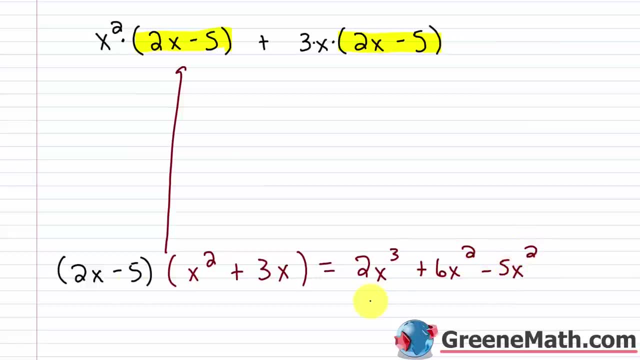 The inner would be minus 5x squared. And then the last would be minus 15x. So if I combine like terms, I would end up with 2x cubed, and then plus x squared, and then minus 15x. 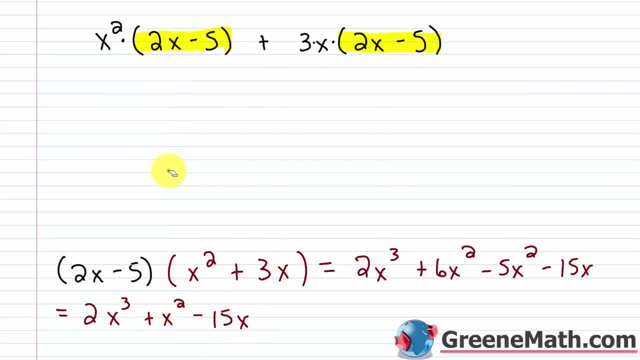 I'm going to show you that you're going to get the same thing up here. Let me kind of erase that real quick. 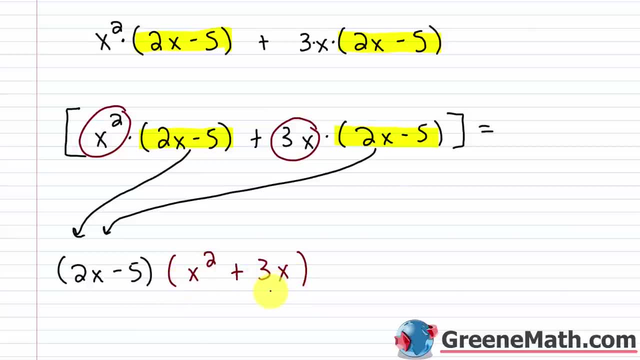 plus 3 x. now we're going to learn later on that we can further factor this and we can pull another x out. right, because that's common to each term here. but for right now, let's not even worry about that. okay, let's just keep it as it is. 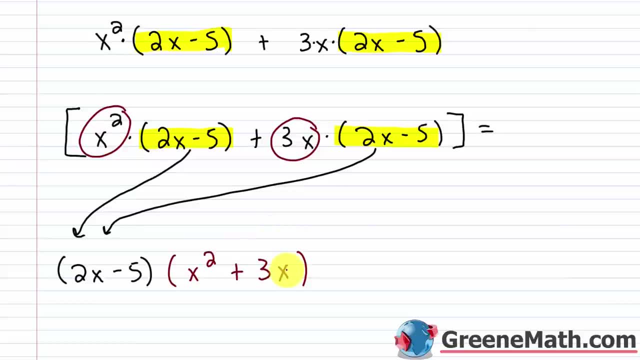 so that is what factoring by grouping is going to entail. we're going to pull out a common binomial factor and you're going to see that kind of moving forward. but before I go on, I want to show something to you. I want to prove to you. 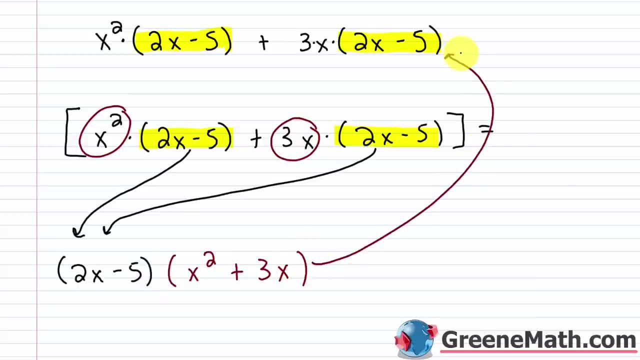 that this is still equal to this, and a lot of you will doubt that, but I want you to notice- let me kind of erase this real fast- I want you to notice that this is nothing more than the way we used to multiply these guys together right before we learned. 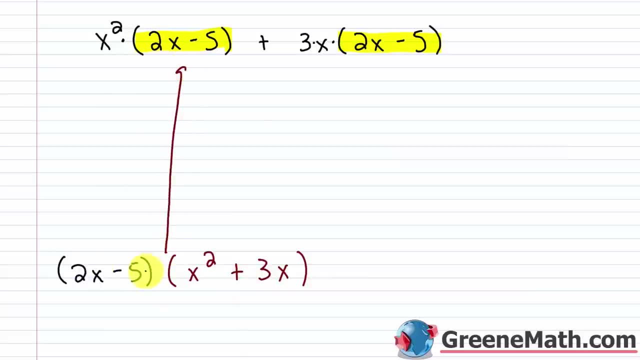 FOIL. we would take this guy right here and we'd multiply it by each term of the second polynomial, so that quantity 2 x minus 5 would get multiplied by x squared, which it is here then plus. we'd have 3 x multiplied by that polynomial. 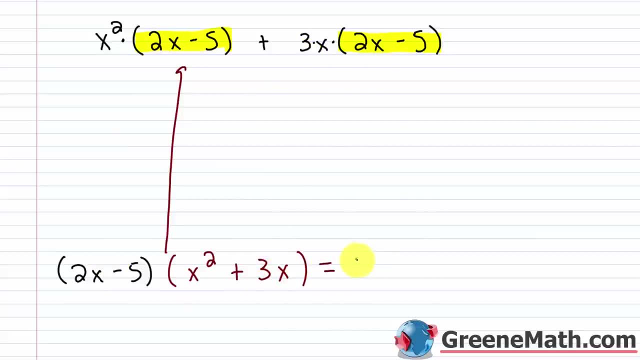 again. so if I did FOIL on this, 2 x times x squared is 2 x cubed. the outer would be what plus 6 x squared, the inner would be minus 5 x squared and then the last would be minus 15 x. so if I combine like terms, 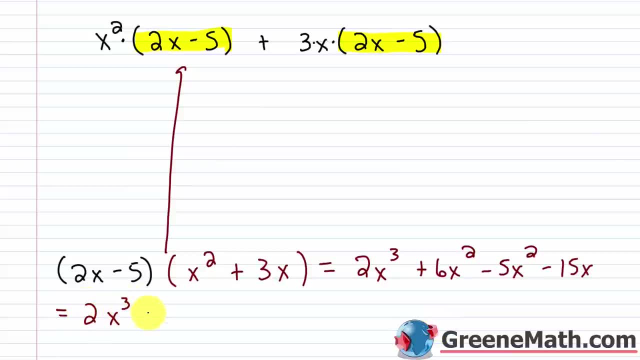 I would end up with 2 x cubed and then plus x squared and then minus 15 x and I'm going to show you that you're going to get the same thing up here. let me kind of erase that real quick. x squared times 2 x is 2 x cubed. 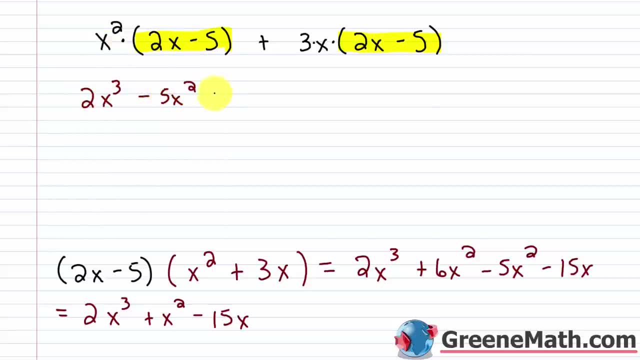 x squared times negative, 5 is minus 5 x squared plus 3 x times 2, x is 6 x squared, and then 3 x times negative, 5 is minus 15 x. so if I combine like terms here again I'm going to get. 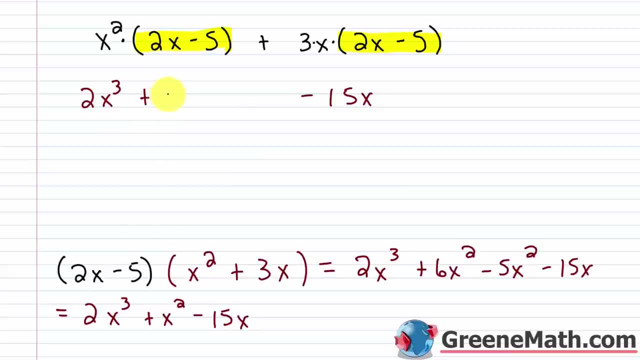 plus x squared in the middle. so 2 x cubed plus x squared minus 15 x. again 2 x cubed plus x squared minus 15 x. alright, so let's scroll down. now we're going to talk about what factoring by grouping is. 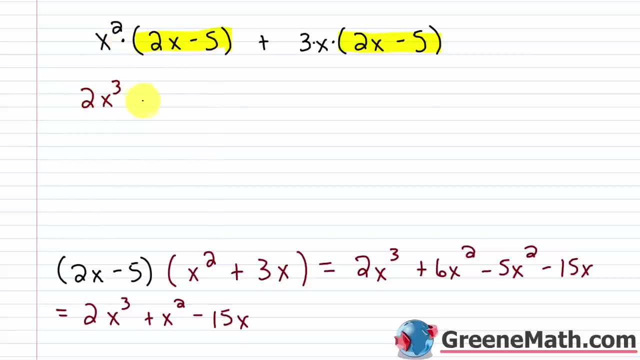 x squared times 2x is 2x cubed. x squared times negative 5 is minus 5x squared. And plus 3x times 2x is 6x squared. 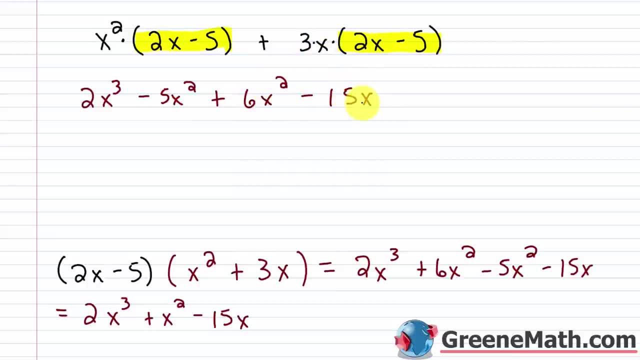 And then 3x times negative 5 is minus 15x. 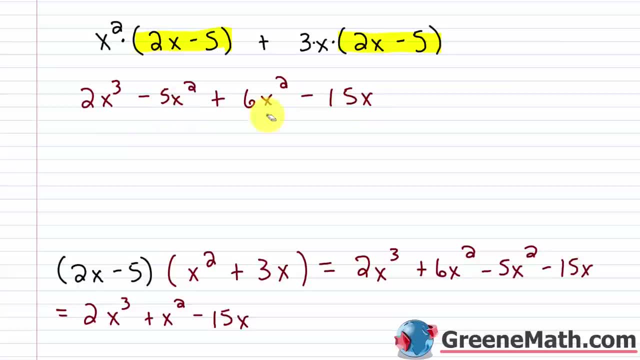 So if I combine like terms here, again, I'm going to get plus x squared in the middle. 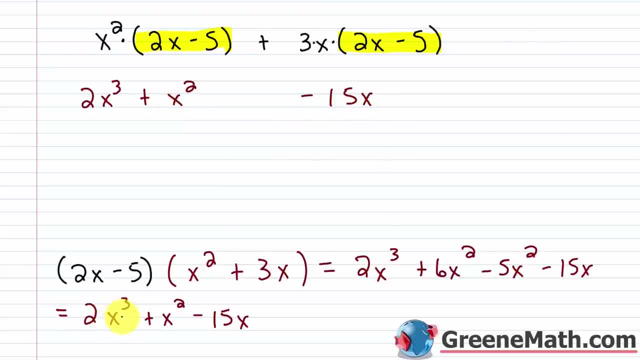 So 2x cubed plus x squared minus 15x. Again, 2x cubed plus x squared minus 15x. All right. So let's scroll down now. 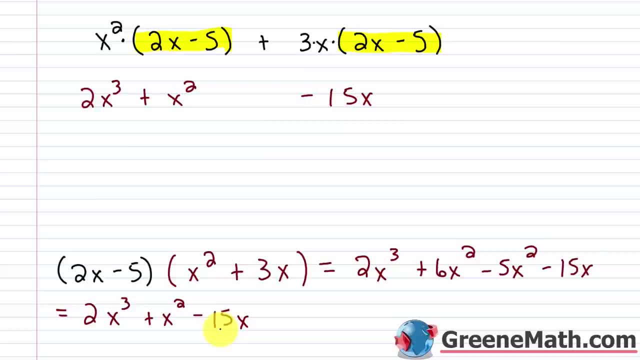 We're going to talk about what factoring by grouping is and how you execute that process. All right. 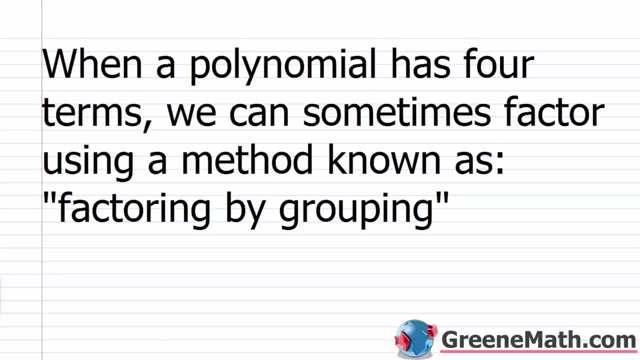 So when a polynomial has four terms, we can sometimes factor using a method known as factoring by grouping. And when we say grouping, we're just putting it into two different groups. 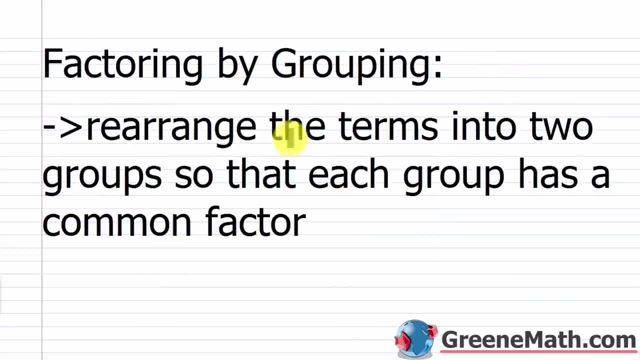 So I'm going to show you that right now. So we're going to rearrange the terms into two groups. Again, two groups. 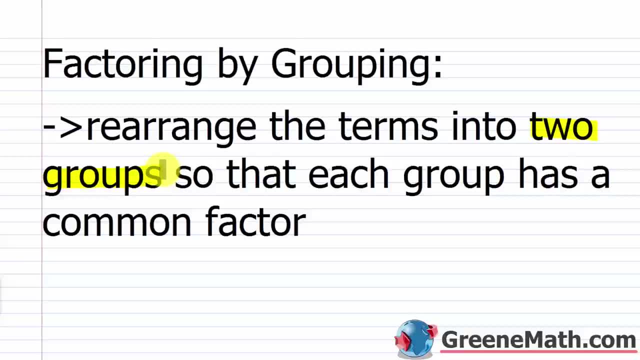 And since there's four groups, and since there's four terms in the polynomial, we have two groups of two terms each. 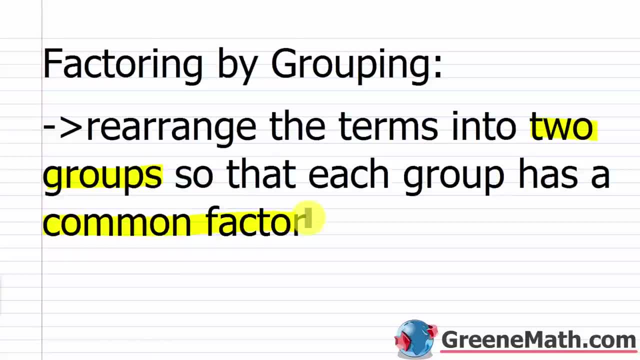 And we're going to do that so that each group has a common factor. And in some cases, the common factor might be 1 or negative 1. 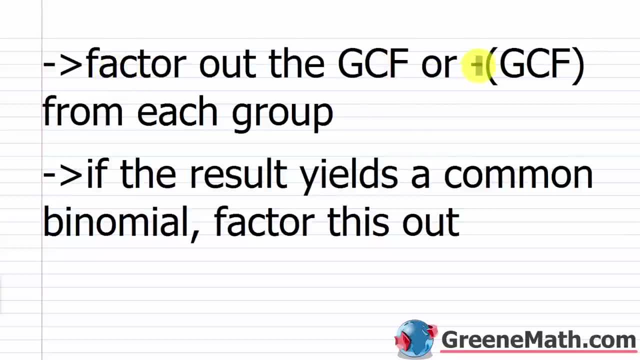 So then the next thing we want to do is factor out the GCF. Or again, in some cases, it might be the negative of the GCF from each group. 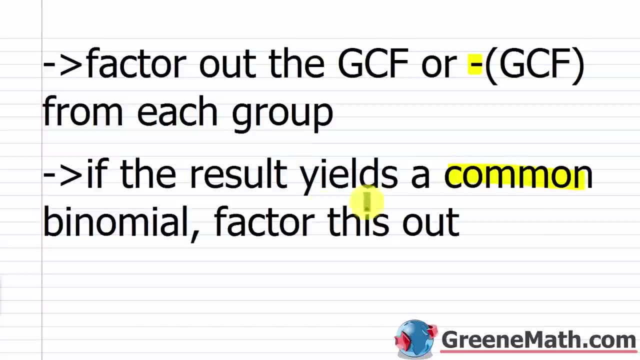 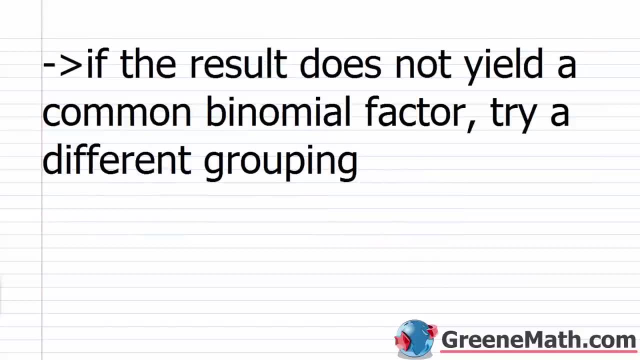 Then if the result yields a common binomial, just like we saw in that example we looked at a minute ago, we want to factor this out. If the result does not yield a common binomial factor, 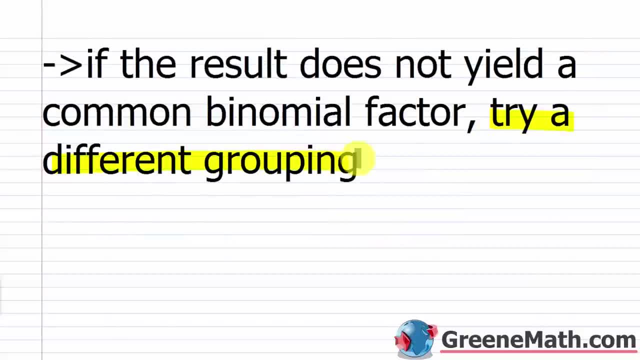 you want to try a different grouping. So you might need to rearrange your terms and set it up into another two groups of two and just try again. 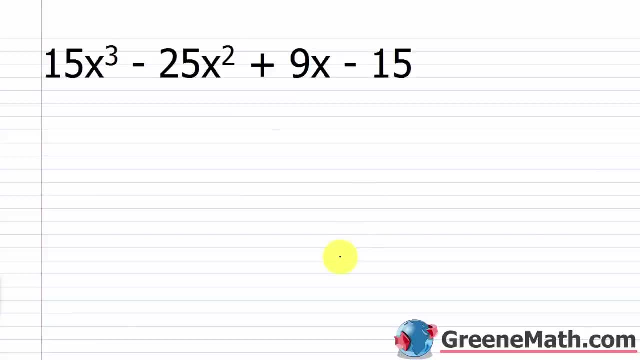 All right, so let's take a look at the first one. So I have 15x cubed minus 25x squared plus 9x minus 15. 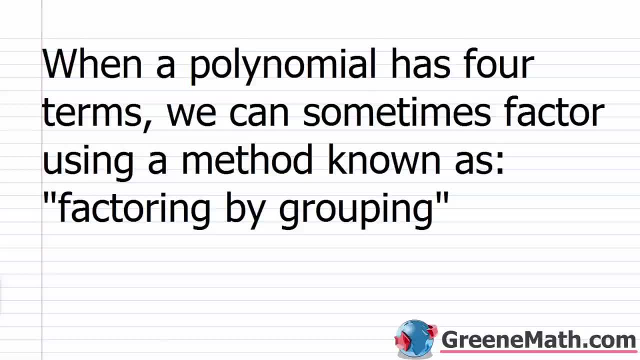 and how you execute that process. alright. so when a polynomial has four terms, we can sometimes factor using a method known as factoring by grouping, and when we say grouping, we're just putting it into two different groups. so I'm going to show you that right now. 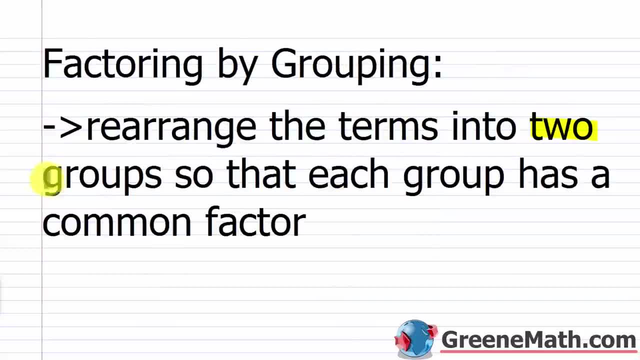 so we're going to rearrange the terms into two groups- again two groups and since there's four terms in the polynomial, we have two groups of two terms each, and we're going to do that so that each group has a common factor and in some cases, the 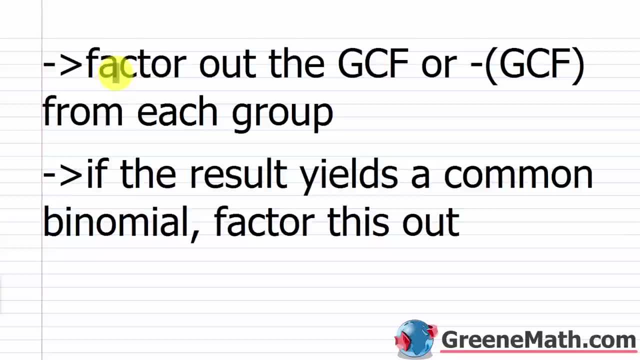 common factor might be one or negative one. so then the next thing we want to do is factor out the GCF- or again, in some cases it might be the negative- of the GCF from each group. then, if the result yields a common binomial, just like we saw in that example we looked at a minute ago, 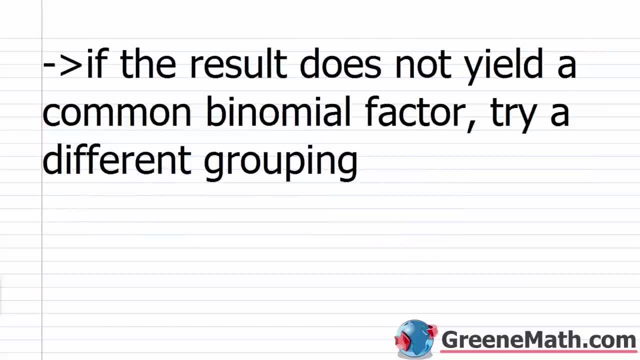 we want to factor this out. if the result does not yield a common binomial factor, you want to try a different grouping, so you might need to rearrange your terms and set it up into another two groups of two and just try again. alright, so let's take a look at the first one. 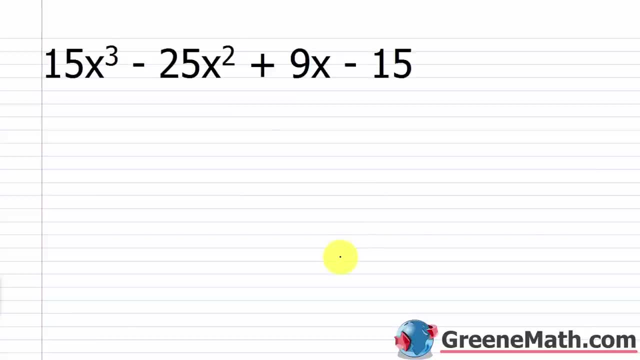 so I have 15x cubed minus 25x squared, plus 9x minus 15. so the first thing I always do is I try to think about if I set it up into two groups of two just as they are, could I pull something common out from each? 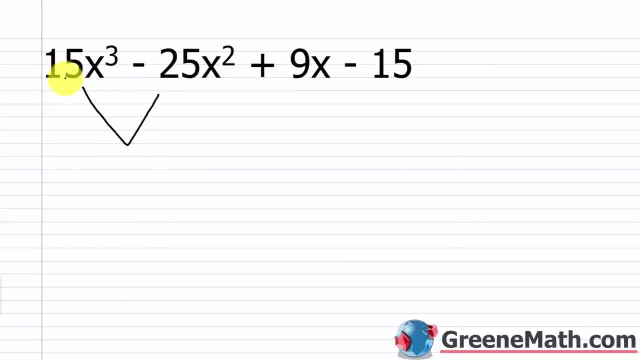 so if I look at these two terms- and I made them into a group- I see they have a five- that's common, and an x squared. that's common, so I could pull that out. if I look at these two, they both have a three in common. so let's go ahead and try that. 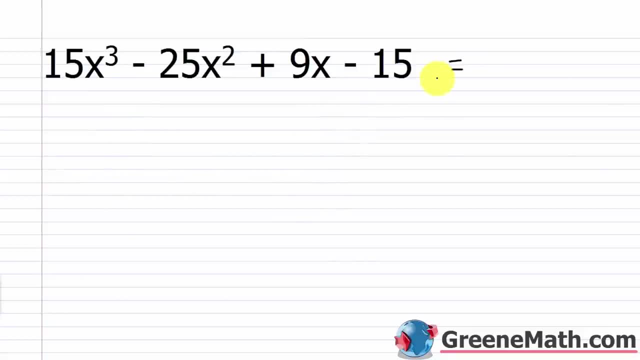 setting this up into again two groups of two, with this being 15x cubed minus 25x squared. let's make that into a group, then plus we'll have a group of 9x minus 15 and again, I already told you the GCF for each for this. 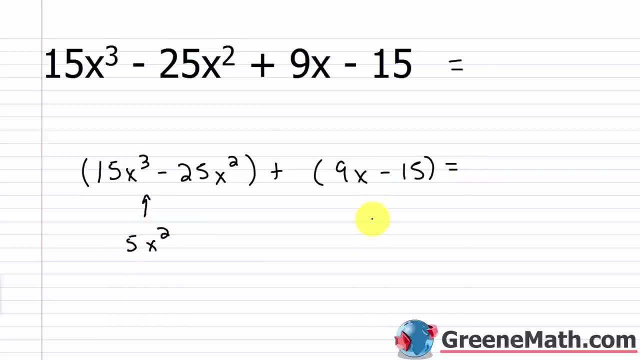 one, it's what it's 5x squared for this one, it's three. so let's pull that out from each one. so if I pulled out a 5x squared from here, what would I have left inside? 15x cubed divided by 5x squared would. 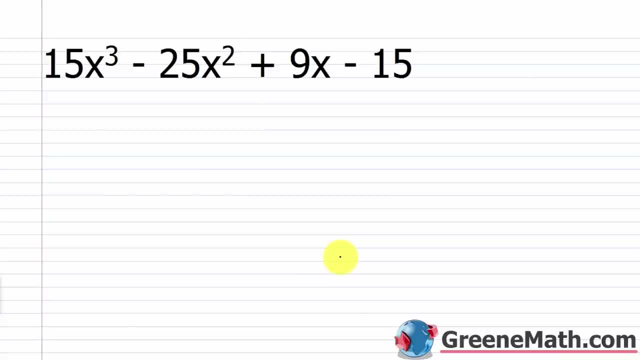 So the first thing I always do is I try to think about if I set it up into two groups of two, just as they are, could I pull something common out from each? So if I look at these two terms and I made them into a group, I see they have a 5 that's common and an x squared that's common. So I could pull that out. 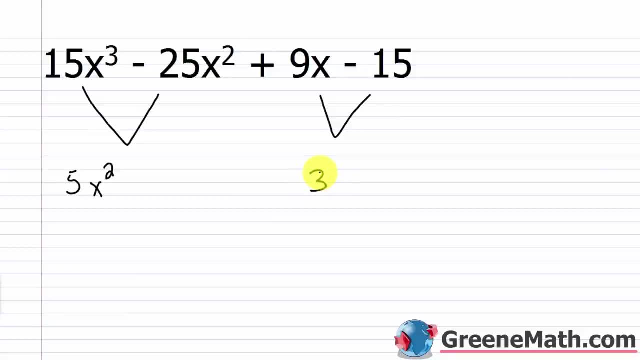 If I look at these two, they both have a 3 in common. So let's go ahead and try that, setting this up into, again, two groups of two, 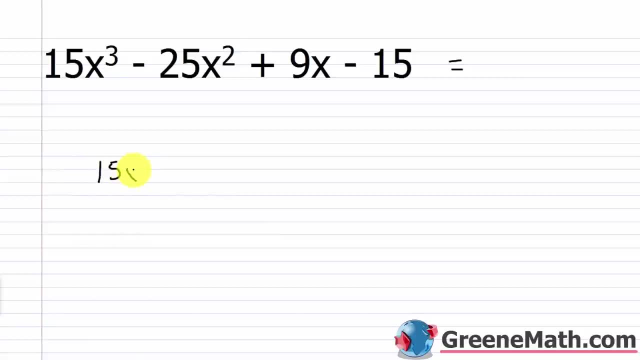 with this being 15x cubed minus 25x squared. Let's make that into a group. Then plus, we'll have a group of 9x minus 15x. 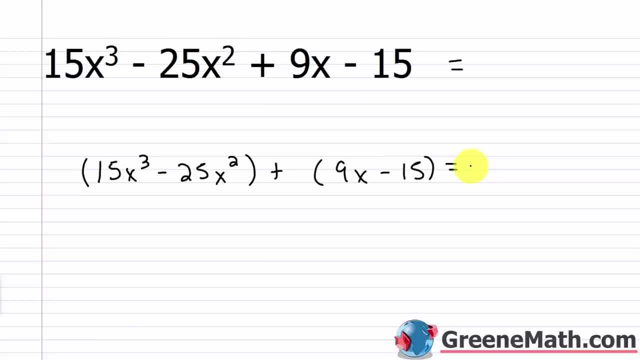 And again, I already told you the GCF for each. For this one, it's what? It's 5x squared. 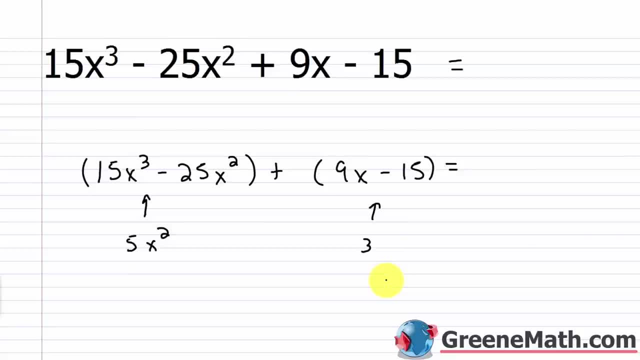 For this one, it's 3. So let's pull that out from each one. So if I pulled out a 5x squared from here, what would I have left inside? 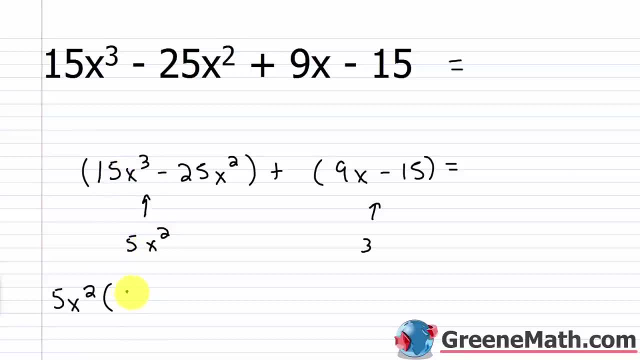 15x cubed divided by 5x squared would be 3x. Then I have the minus. 25x squared over 5x squared is 5. 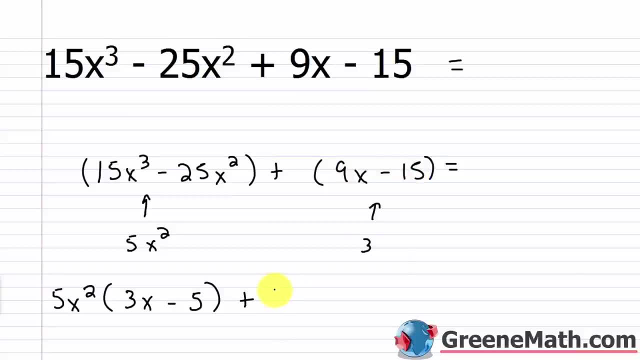 And then plus. If I pulled a 3 out from here, 9x divided by 3 would be 3x. 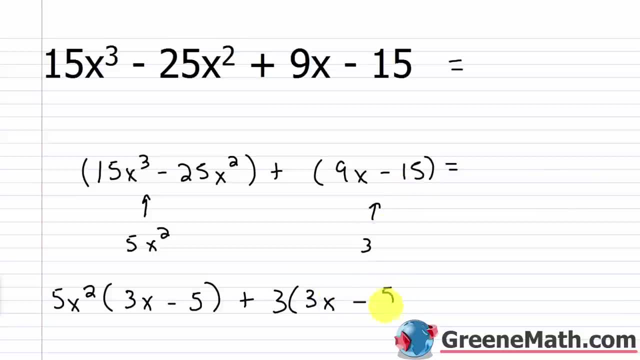 Then minus. 15 divided by 3 would be 5. 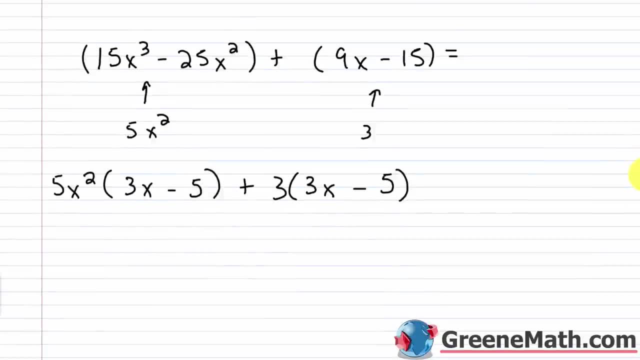 So we can see that immediately we have a common binomial factor. We have 3x minus 5 and we have 3x minus 5. So we're going to pull this out. We're going to pull this out. So again, imagine I have parentheses around the whole thing. And I pulled out the 3x. Minus 5. What would be left inside? 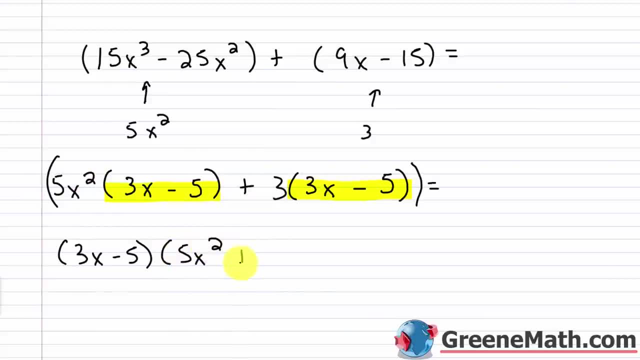 Well, I'd have a 5x squared plus a 3. 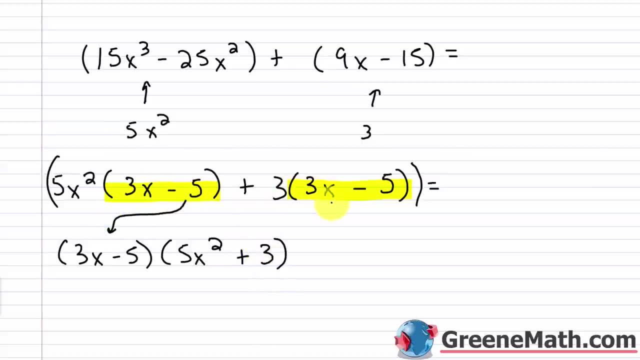 Because this was pulled out. I can just kind of draw an arrow down here. That's pulled out, put outside. That's what's left inside. The 5x squared plus the 3. 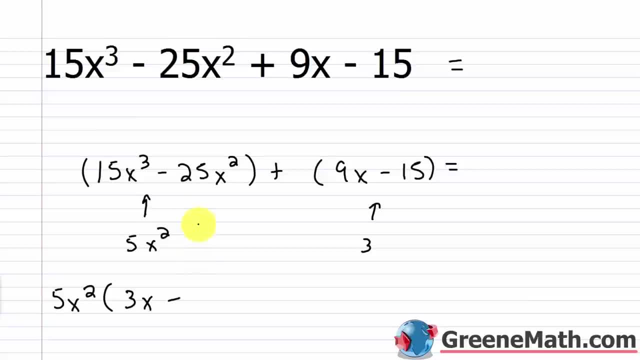 be 3x, then I have the minus 25x squared over. 5x squared is 5 and then plus. if I pulled a 3 out from here, 9x divided by 3 would be 3x, then minus 15 divided by 3 would. 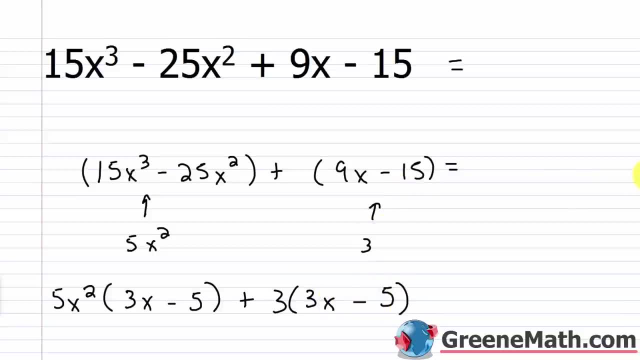 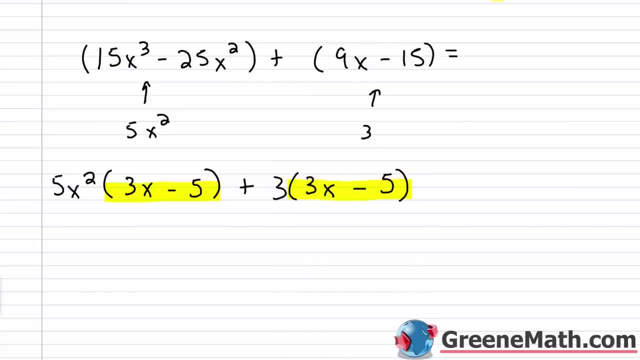 be 5, so we could see that immediately. we have a common binomial factor, we have 3x minus 5 and we have 3x minus 5, so we're going to pull this out. so again, imagine I have parentheses around the whole thing. 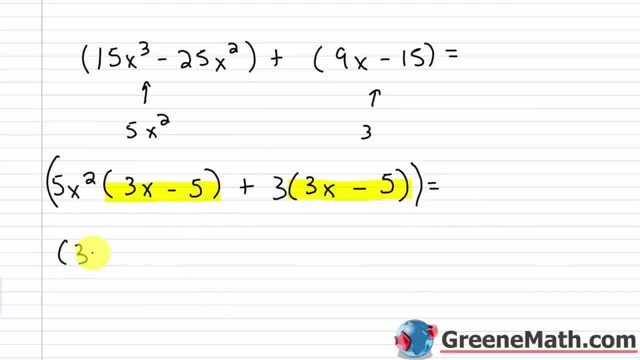 and I pulled out the 3x minus 5, what would be left inside? well, I'd have a 5x squared plus a 3, because this was pulled out. I can just kind of draw an arrow down here. that's pulled out, put outside, that's what's left. 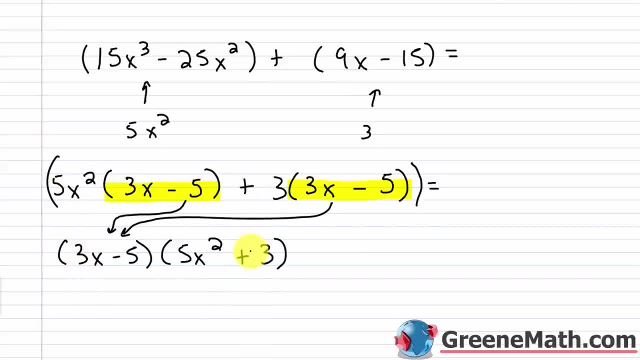 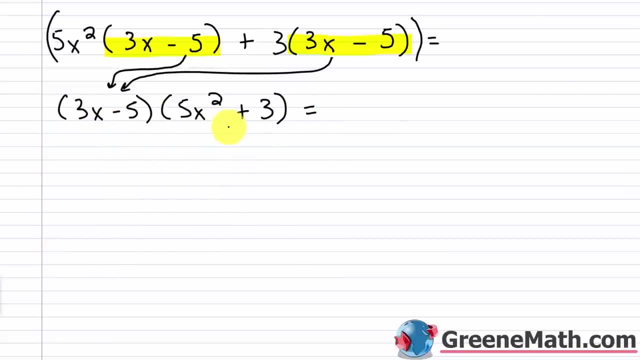 inside the 5x squared plus the 3. so we have successfully factored this by grouping. so what we can do is use FOIL here and we can prove that these two would multiply together to give us that original four term polynomial. so 3x times 5x. 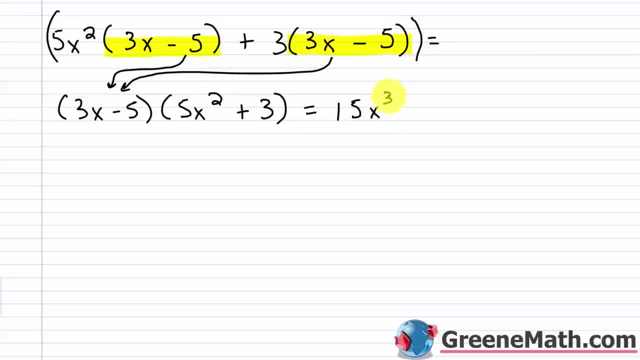 squared is 15x cubed, then 3x times 3 is plus 9x, then negative 5 times 5x. squared is minus 25x. squared, then negative 5 times 3 is negative 15 and if I reorder the terms, I get 15x. 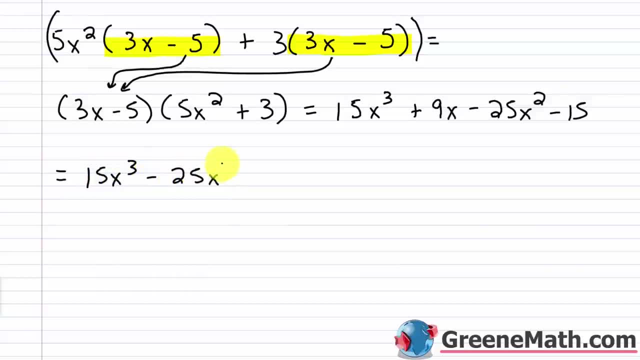 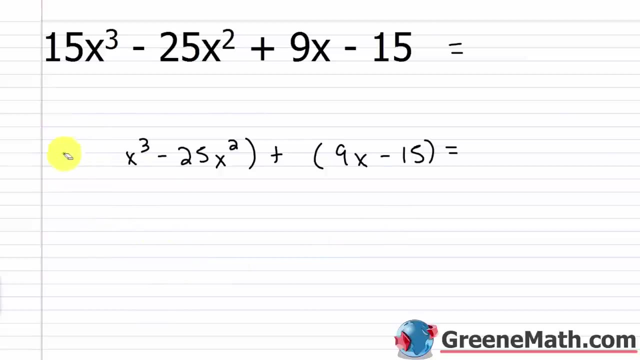 cubed minus 25x, squared plus 9x minus 15, which is exactly what we started with. now let me erase this real quick and I want to show you that this would also work with a different grouping. so let's say you decided to reorder the terms. 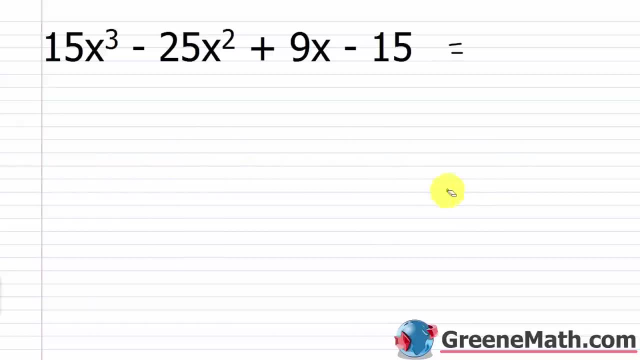 and you said that you wanted to look at, I don't know, 15x cubed plus 9x. let's say that's a group, because you can see that there's a 3x that's common. there's a 3x that's common. and then 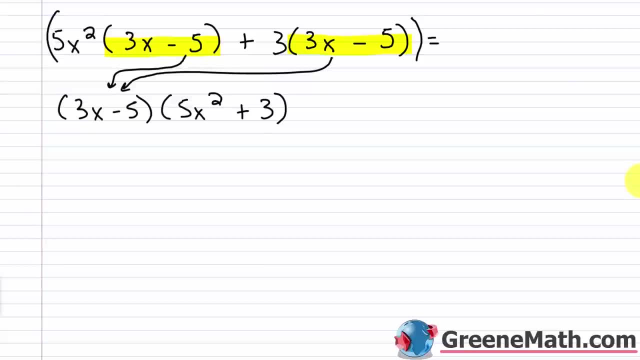 So we have successfully factored this by grouping. So what we can do is use FOIL here. 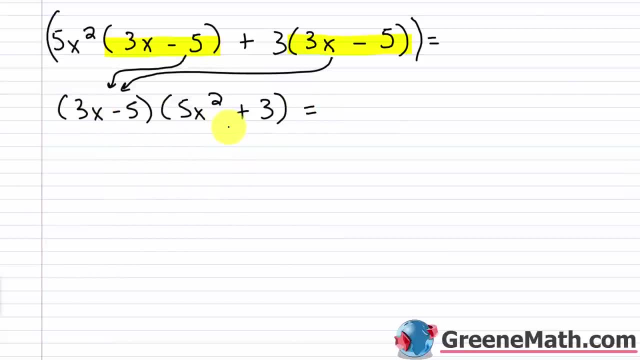 And we can prove that these two would multiply together to give us that original four-term polynomial. So 3x times 5x squared is 15x cubed. Then 3x times 3 is plus 9x. Then negative 5 times 5x squared is minus 25x squared. Then negative 5 times 3 is negative 15. And if I reorder the terms, I get 15x cubed minus 25x squared plus 9x minus 15. Which is exactly what we started with. 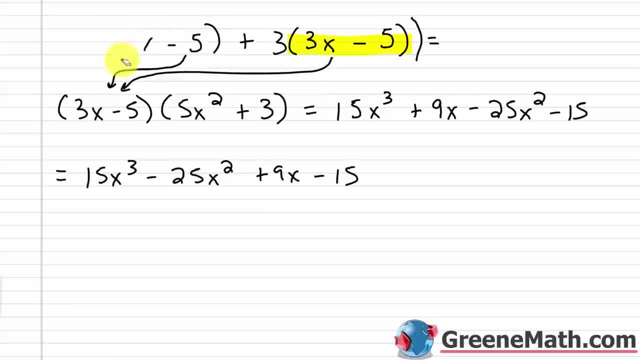 Now let me erase this real quick. And I want to show you that this would also work with a different grouping. 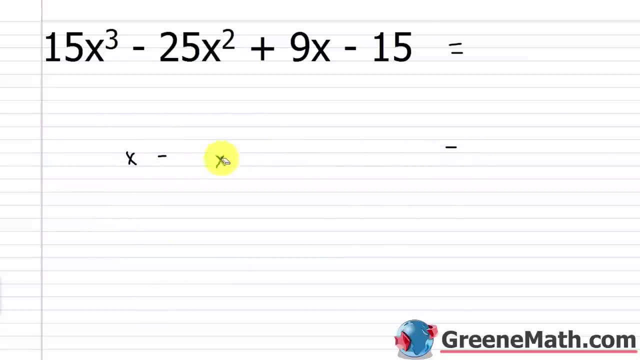 So let's say you decided to reorder the terms. And you said that you wanted to look at, I don't know, 15x cubed plus 9x. Let's say that's a group. Because you can see that there's a 3x that's common. There's a 3x that's common. And then you have another group that's negative 25x squared and minus 15. And what's common here, I'm going to pull out a negative and then a 5. 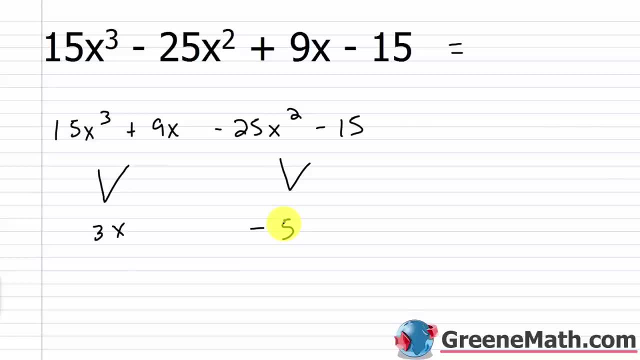 So negative 5 is common to both. So if we do that, what would we get? 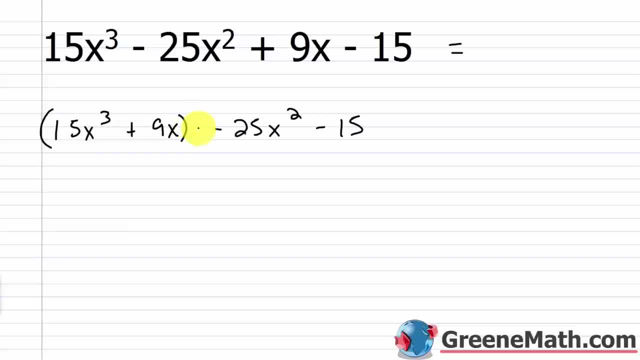 So let's put parentheses around each. Let's put parentheses around each. 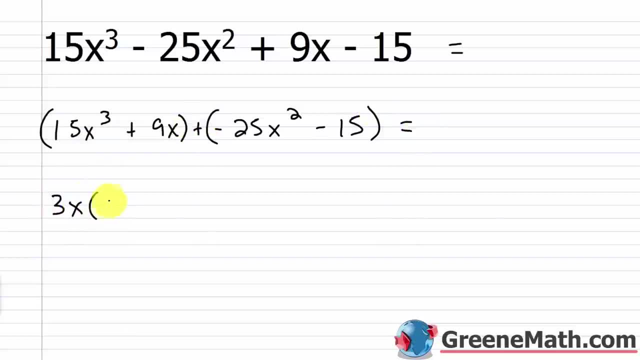 And again, I'm going to pull out a 3x from here. So 3x times, inside I would have a 5x squared plus a 3. And then from here, remember, I'm going to pull out a negative 5. So I'd have plus and I'm going to have a negative 5 out in front. And then inside I'd have what? 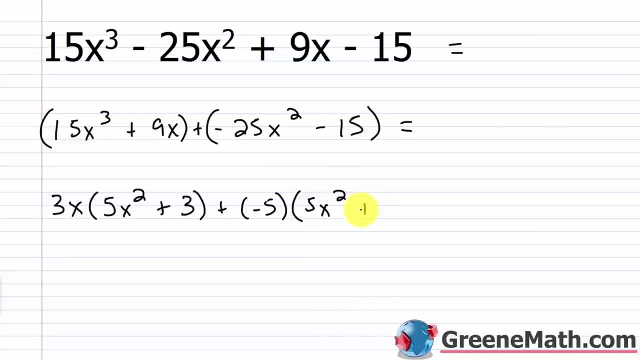 I'd have 5x squared plus 3. 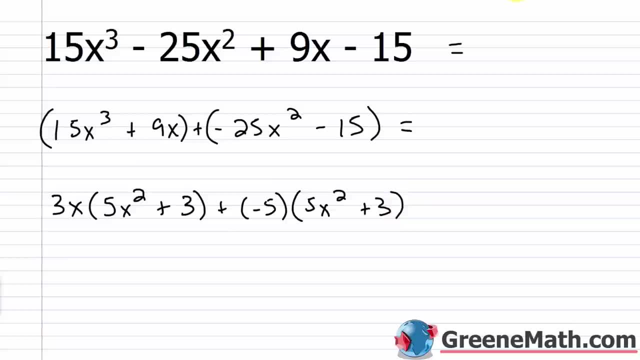 Now I didn't have the same binomial factor. But what's interesting is that if I look at this here and I pulled this out, what I'm going to end up with is the same thing in the end. 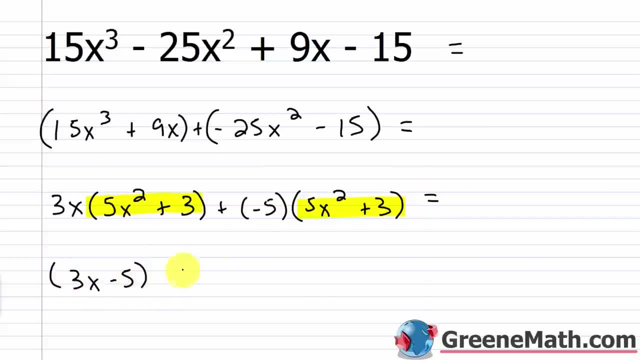 I have what? I have 3x minus 5, which is what I ended up pulling out last time, 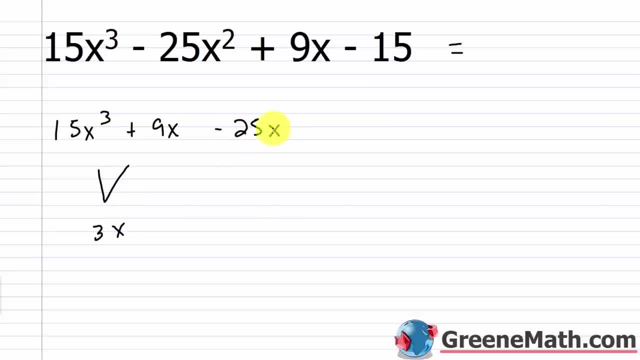 you have another group that's negative 25x squared and minus 15. and what's common here? I'm going to pull out a negative and then a 5. so negative 5 is common to both. so if we do that, what would we get? so let's. 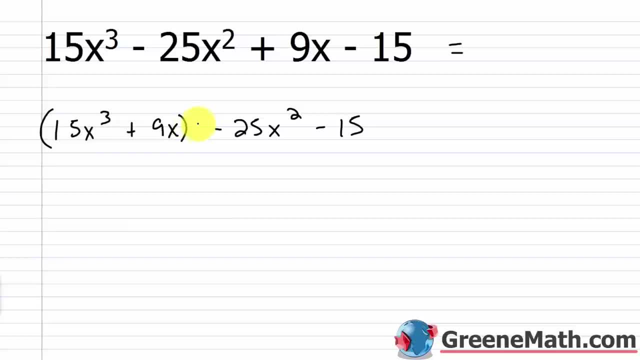 put parentheses around each. put parentheses around each and again. I'm going to pull out a 3x from here, so 3x times inside I would have a 5x squared plus a 3, and then from here- remember, I'm going to pull out a negative. 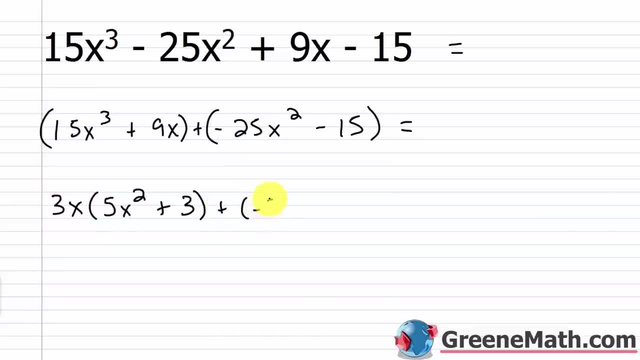 5. so I'd have plus and I'm going to have a negative 5 out in front and then inside I'd have what I'd have: 5x squared plus 3. now I didn't have the same binomial factor, but what's interesting is that, if I look, 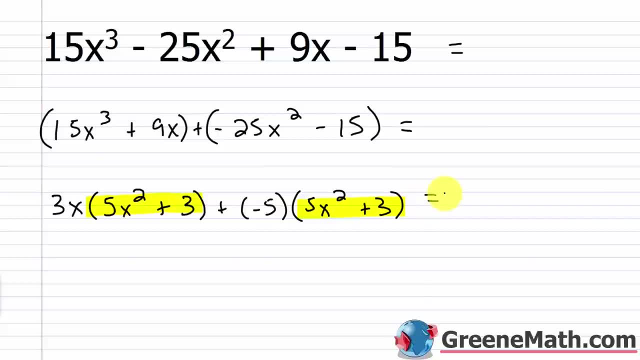 at this here and I pulled this out. what I'm going to end up with is the same thing. in the end, I have what I have: 3x minus 5, which is what I ended up pulling out last time, times 5x squared plus 3. so 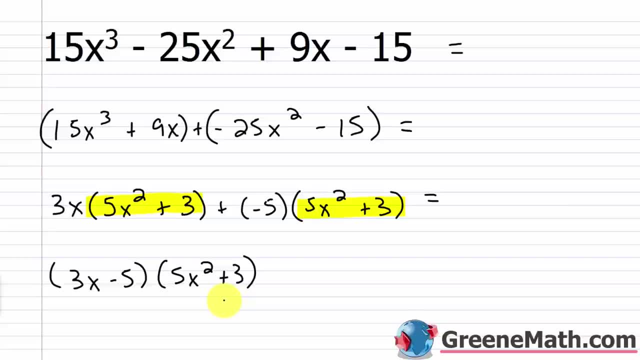 I end up with the same two binomials, right, but it's a little bit different how I got there. now I want to show you one last thing. if you had chosen, if you had chosen to do- let's say 15x cubed minus 15, let's say that's one group. 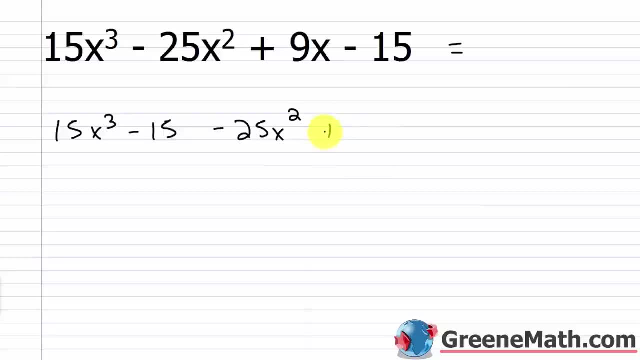 and then negative 25x squared plus 9x, let's say that's another group. this would not yield a common binomial factor. so what's common here would be what it would be 15. so if I pull out a 15 here, I would have x cubed minus. 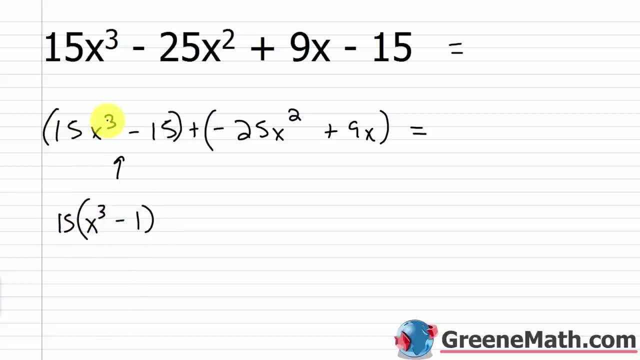 1 inside the parentheses right. 15x cubed divided by 15 would just be x cubed and then negative. 15 divided by 15 would be negative 1. then kind of thinking about over here I could pull out an x or negative x, however you want to do that. 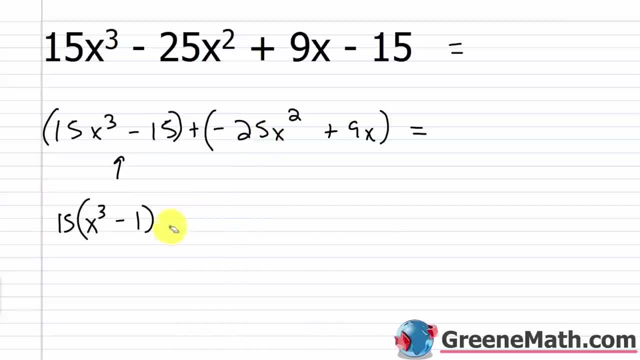 wouldn't matter either way. so let's pull out a negative x, so let's put minus x times inside of here we'd still have 25x, and then here we'd have a minus 9. so you can see that you don't have a common binomial factor here. 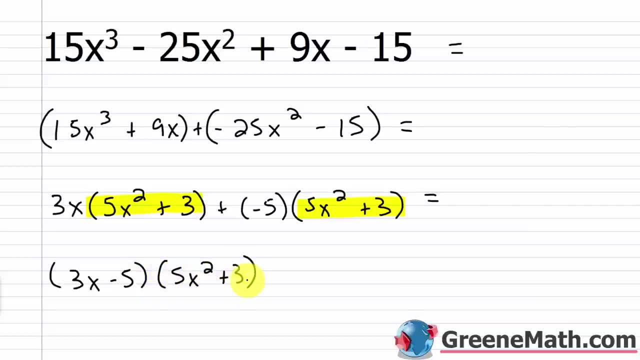 times 5x squared plus 3. So I end up with the same two binomials, right? But it's a little bit different how I got there. 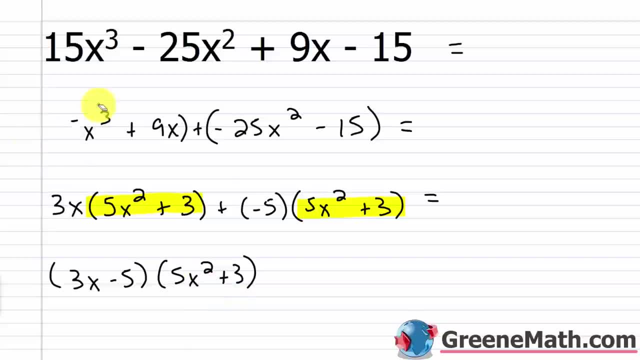 Now I want to show you one last thing. If you had chosen to do, let's say, 15x cubed minus 15. 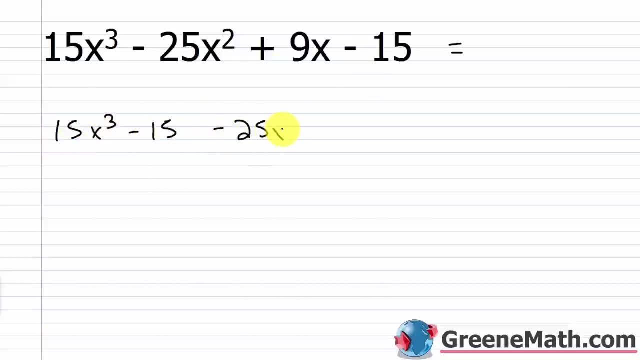 Let's say that's one group. And then negative 25x squared plus 9x. Let's say that's another group. 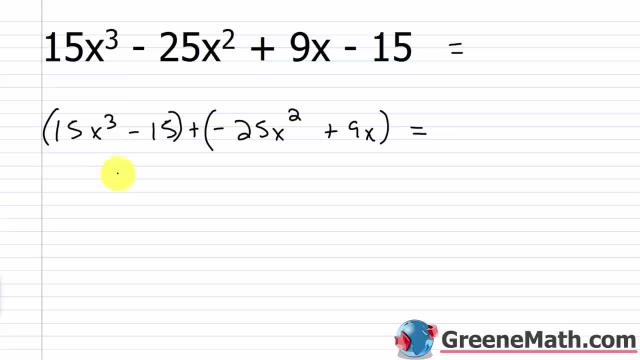 This would not yield a common binomial factor. So what's common here would be what? It would be 15. So if I pull out a 15 here, I would have x cubed minus 1 inside the parentheses. Right? 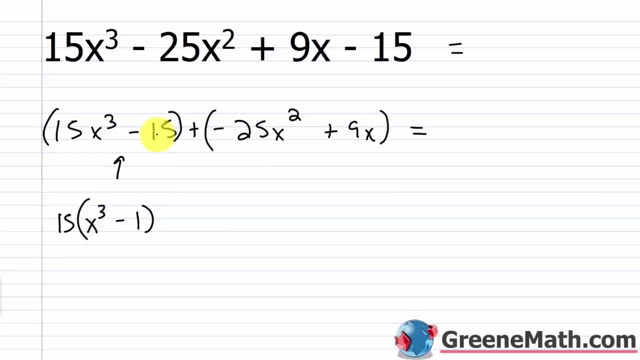 15x cubed divided by 15 would just be x cubed. And then negative 15 divided by 15 would be negative 1. So if I'm thinking about over here, I could pull out an x or a negative x, however you want to do that. It wouldn't matter either way. So let's pull out a negative x. So let's put minus x times. Inside of here we'd still have 25x. 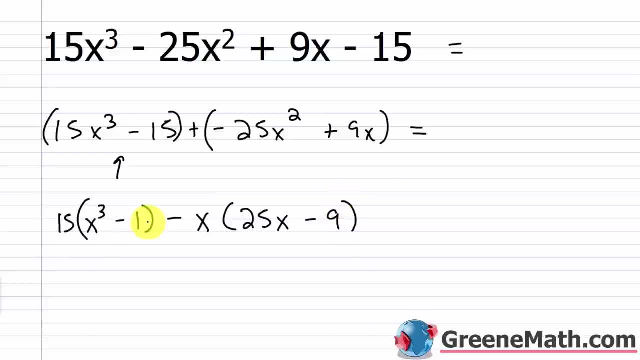 And then here we'd have a minus 9. So you can see that you don't have a common binomial factor here. You have x cubed minus 1 and you have 25x minus 9. Not a common binomial factor. So this is one of the scenarios where you might have set it up like that and said, okay, well there's something common to each one that I can pull out. You pull it out. You don't have a common binomial factor. So you have to try a different grouping. Let's take a look at another one. And we'll kind of speed through these now. 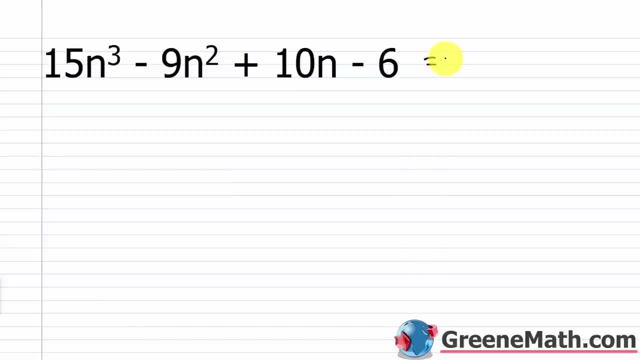 So we have 15n cubed minus 9n squared plus 10n minus 6. So I always like to look at the way they're set up. I start out with these two and these two. So I'll say, okay, what could I pull out of here? Well, I could pull out a 3n squared. What could I pull out of here? I could pull out a 2. 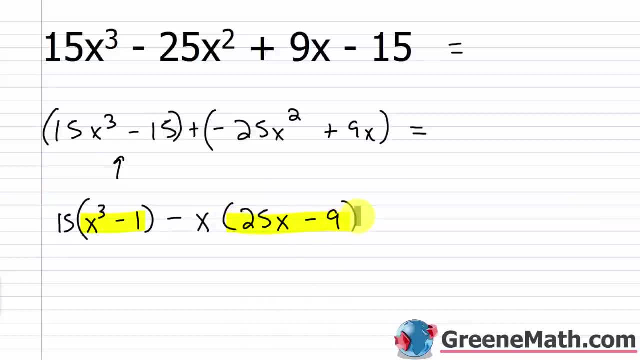 you have x cubed minus 1 and you have 25x minus 9, not a common binomial factor. so this is one of the scenarios where you might have set it up like that and said, okay, well, there's something common to each one that I can pull out. 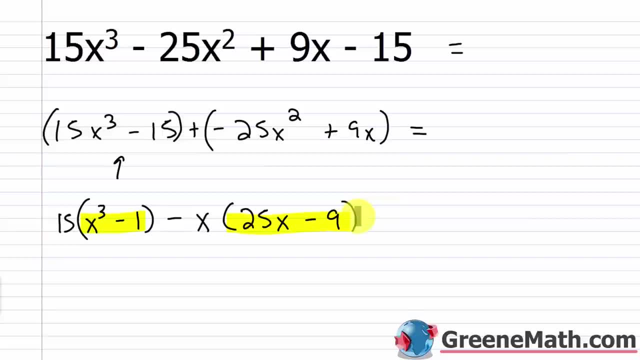 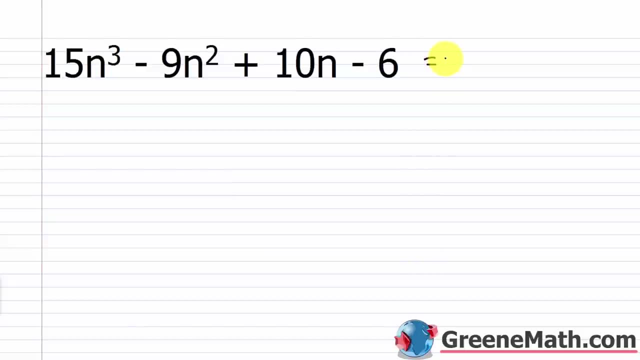 you pull it out, you don't have a common binomial factor, so you have to try a different grouping. let's take a look at another one and we'll kind of speed through these now. so we have 15n cubed minus 9n squared. 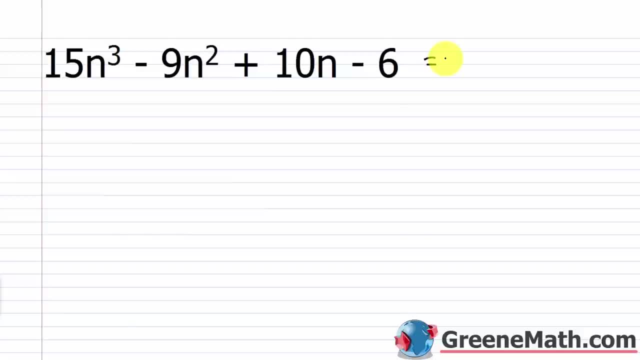 plus 10n minus 6. so I always like to look at the way they're set up. I start out with these two and these two, so I'll say, okay, what could I pull out of here? well, I could pull out a 3n squared. what could I? 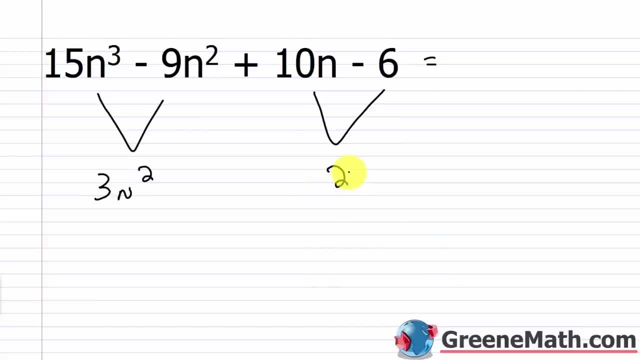 pull out of here? well, I could pull out a 2. so mentally you can kind of look at it and say, well, if I pulled out a 3n squared here, what would I have left in here? well, I'd have a 5n and I'd have. 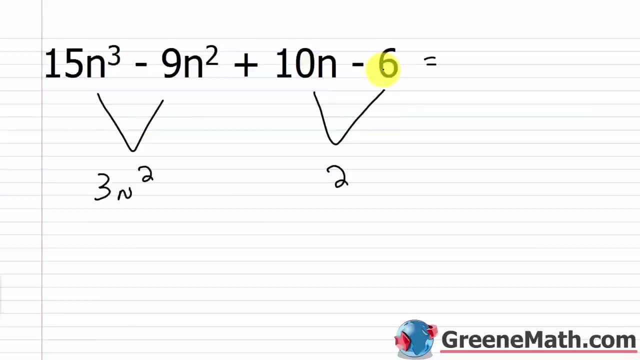 a 3. if I pulled out a 2 here, I'd have a 5n and I'd have a 3, so I already know that's going to work out right. that's what you're going to do, kind of moving forward. you're going to kind of do the groups here. 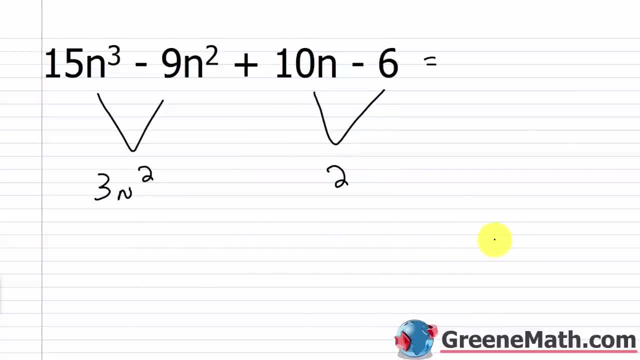 you're not going to go through all the tedious process of writing everything out. you're going to do it mentally and then figure out what group is going to work. so I'm going to pull out again a 3n squared from that first group and that's going to give me 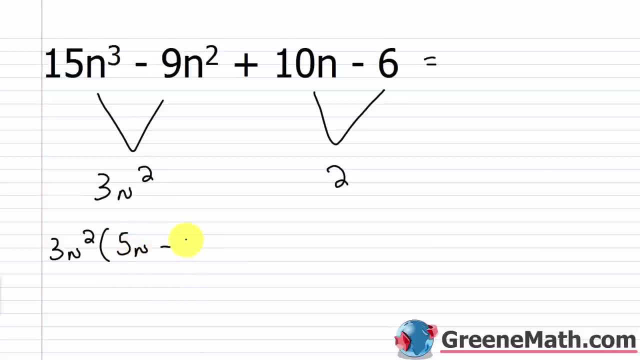 a 5n minus a 3, and then plus, I'm going to pull out a 2 and that's going to give me a 5n minus a 3. so I have my common binomial factor here, which is 5n minus 3. 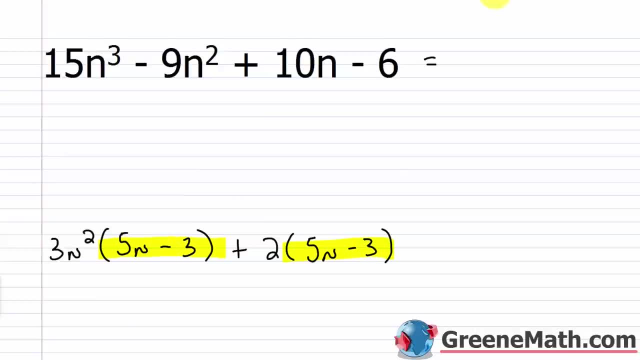 5n minus 3. and if I pull that guy out, what am I going to have? so I'd have 5n minus 3 times what would be left if I pulled out a 5n minus 3 here. I'd have 3n squared. 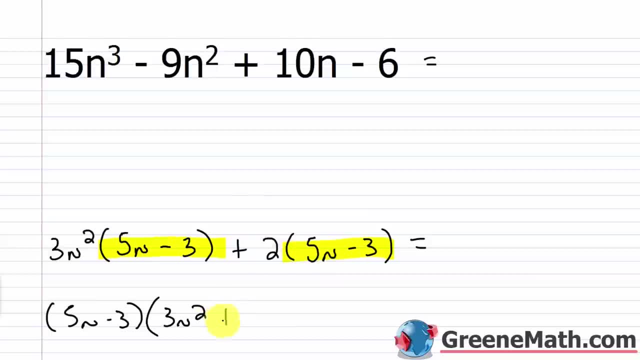 if I pulled out a 5n minus 3 here, I'd have a 2, so plus 2, and so this is my factored form. I have the quantity 5n minus 3 times the quantity 3n squared plus 2, and in the end 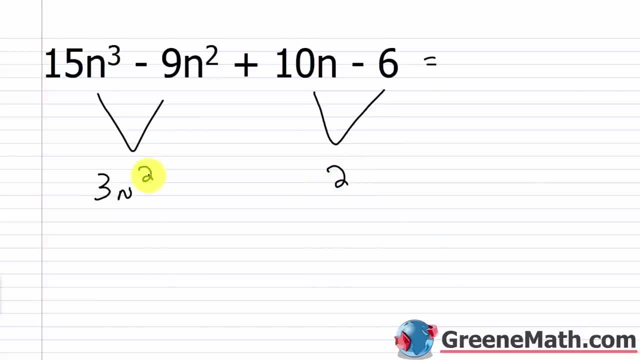 So mentally you can kind of look at it and say, well, if I pulled out a 3n squared here, what would I have left in here? Well, I'd have a 5n and I'd have a 3. If I pulled out a 2 here, I'd have a 5n and I'd have a 3. So I already know that's going to work out, right? That's what you're going to do kind of moving forward. 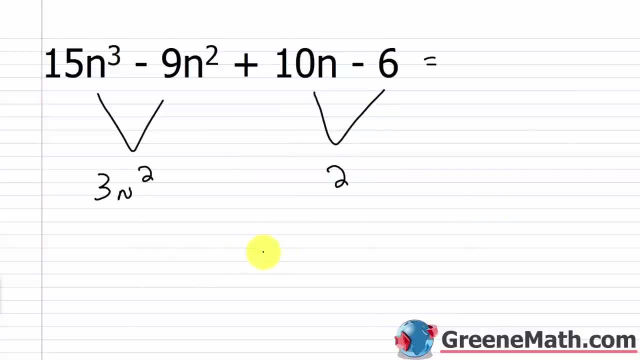 You're going to kind of do the groups here. You're not going to go through all the tedious process of writing everything out and doing it. You're going to do it mentally and then figure out what group is going to work. 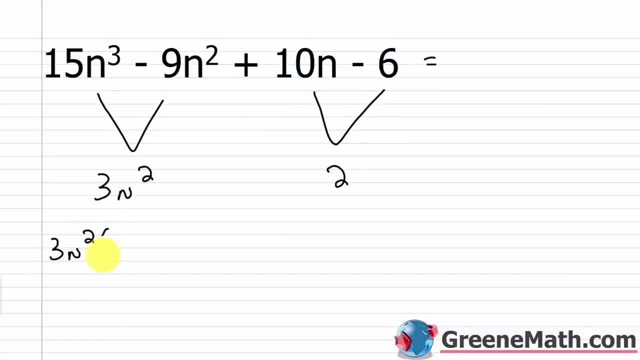 So I'm going to pull out again a 3n squared from that first group. And that's going to give me a 5n minus a 3. And then plus, I'm going to pull out a 2. 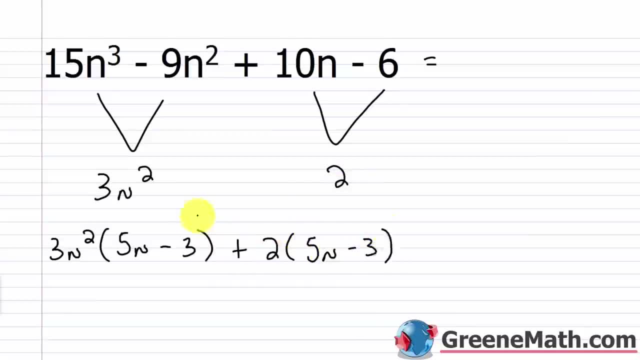 That's going to give me a 5n minus a 3. 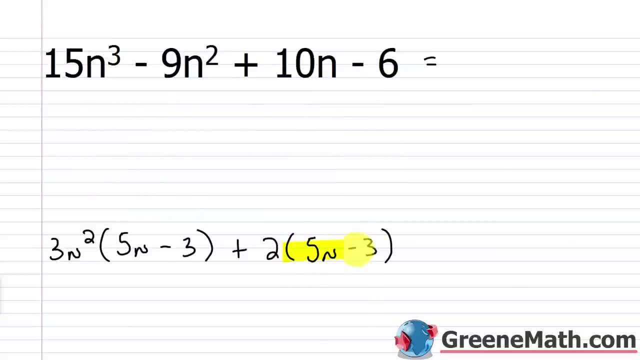 So I have my common binomial factor here, which is 5n minus 3. 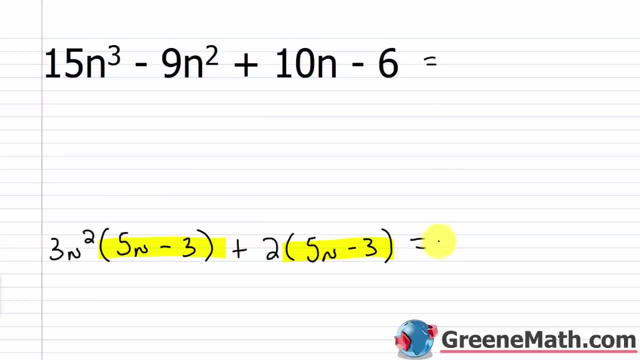 Okay, 5n minus 3. And if I pull that guy out, what am I going to have? 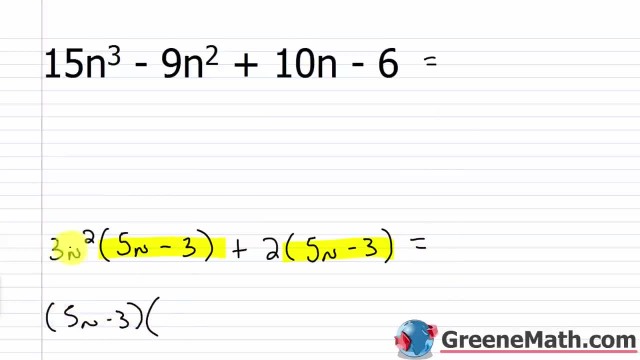 I'm going to have 5n minus 3 times what would be left. 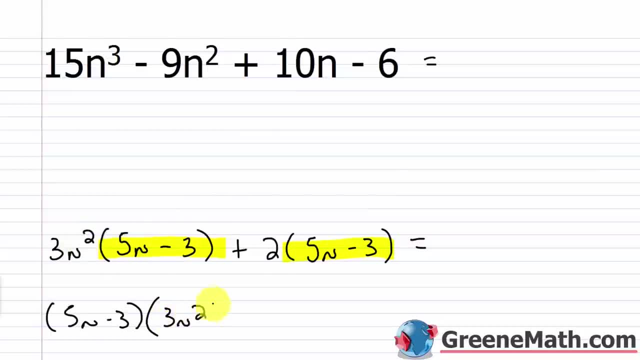 If I pulled out a 5n minus 3 here, I'd have 3n squared. 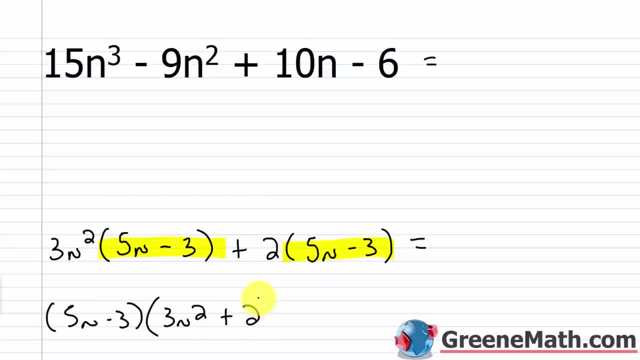 If I pulled out a 5n minus 3 here, I'd have a 2. So plus 2. And so this is my factored form. 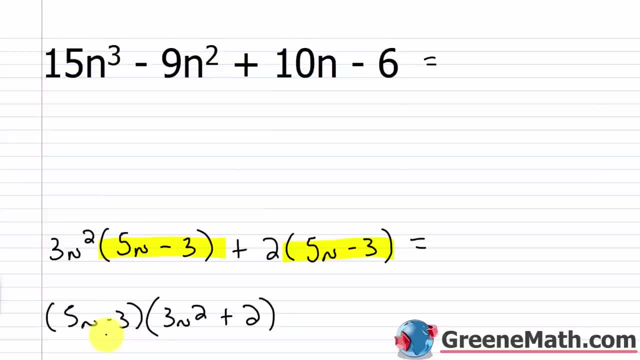 I have the quantity 5n minus 3 times the quantity 3n squared plus 2. And in the interest of time, I'm not going to check it, but if you went back and used FOIL, you would get this four-term polynomial back. 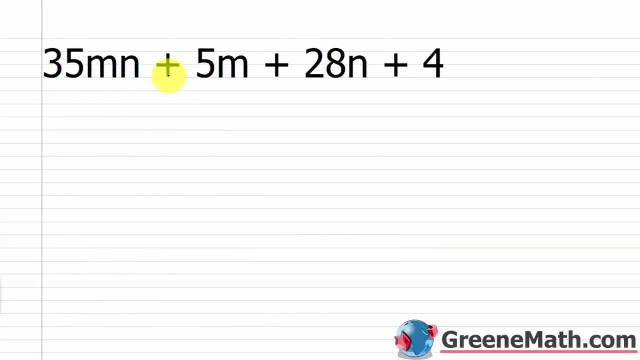 All right, let's take a look at another one. We have 35mn plus 5m, and then we have plus 28n plus 4. 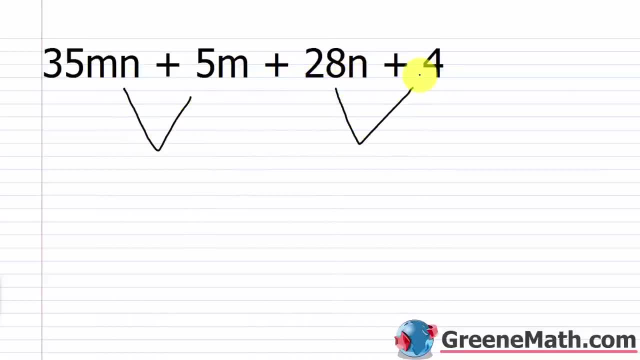 So again, let's check these first two and the last two. 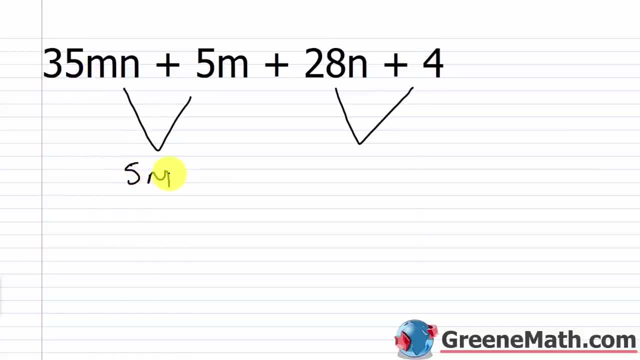 So if I pulled out a 5m, what would I have here? 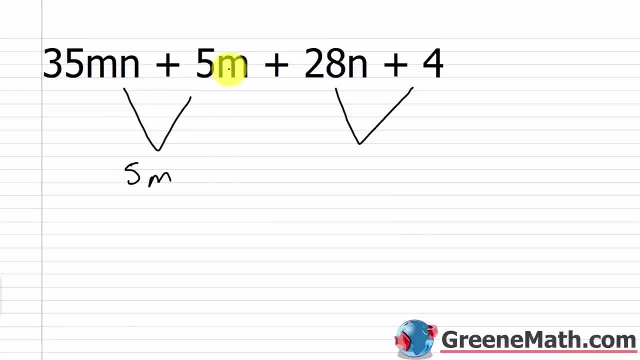 Well, this would be 7n, and this would be 1. If I pulled out what's common to both, which is 4, 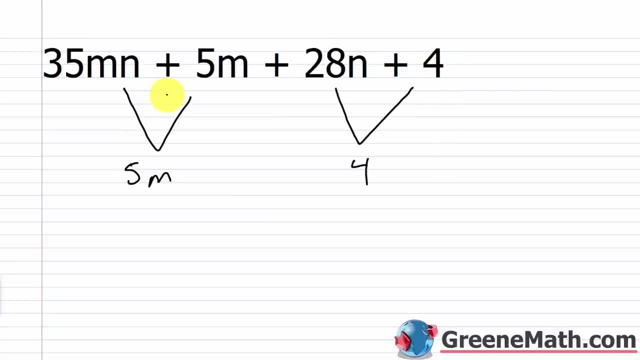 this would be 7n, and this would be 1. So that's exactly what we need. 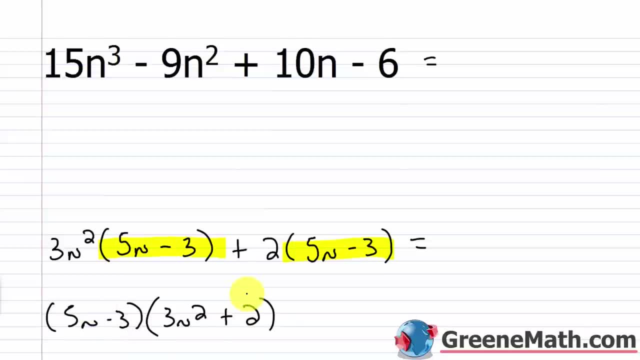 in the interest of time, I'm not going to check it, but if you went back and used FOIL, you would get this four term polynomial back. alright, let's take a look at another one. so we have 35mn plus 5m, and then we have plus 28n. 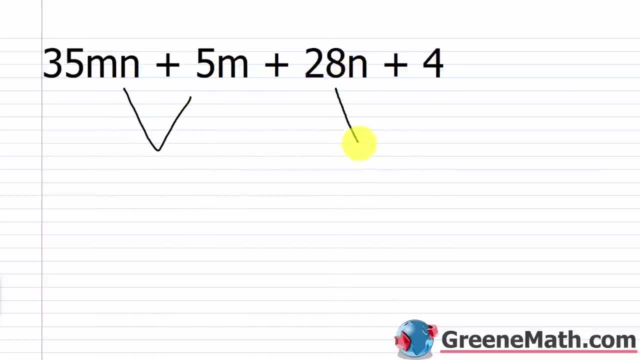 plus 4. so again, let's check these first two and the last two. so if I pulled out a 5m, what would I have here? well, this would be 7n and this would be 1. if I pulled out what's common to both. 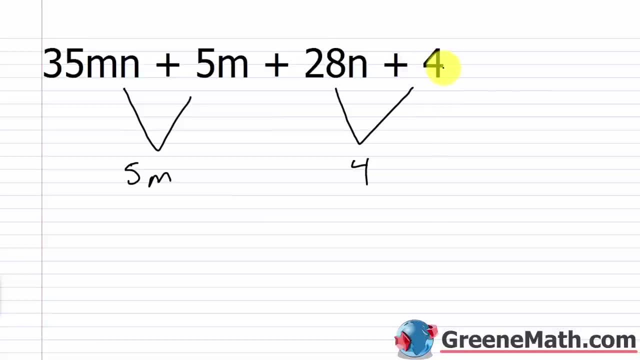 is 4, this would be 7n and this would be 1, so that's exactly what we need. so let's go ahead and do that, so we'll put equals again. in this first one. I'm pulling out a 5m and what's left inside? 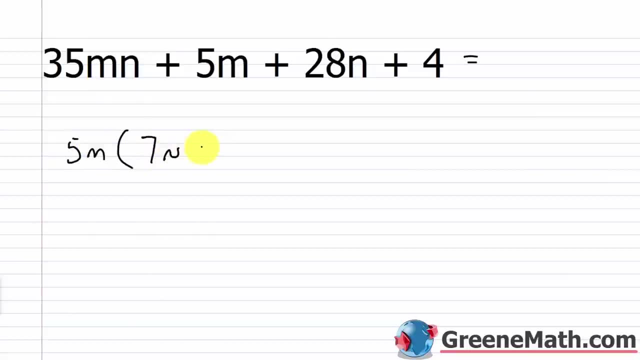 35mn divided by 5m is 7n plus 5m over 5m is 1, plus when I'm pulling out of this group, pulling out a 4. so 28n divided by 4 is 7n plus 4 over 4 is 1. 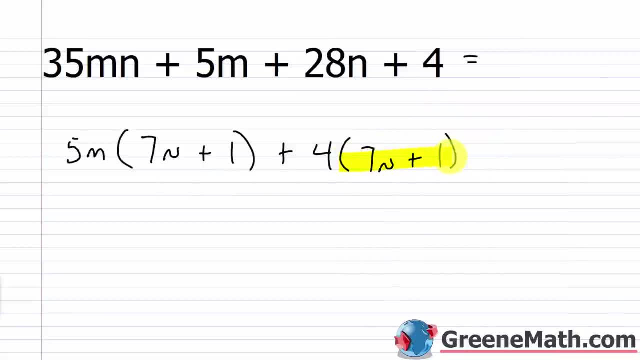 so you can see we have that common binomial factor of 7n plus 1. ok, that quantity there. so if I pulled that out I would have 7n plus 1 outside and then I would have 5m. that's left here, 5m. 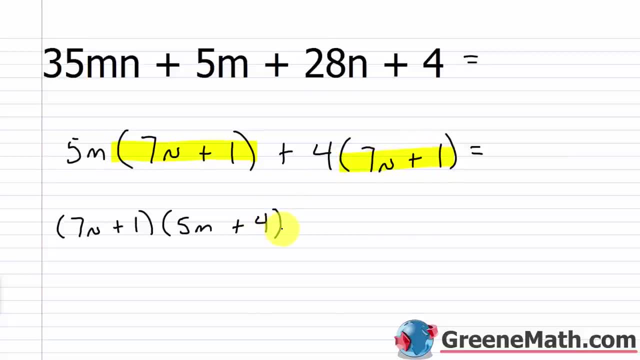 plus. from here this is gone, so I just have a 4. so I'd have the quantity 7n plus 1 times the quantity 5m plus 4, and again, if you use FOIL to check this, you're going to end up with this exact same. 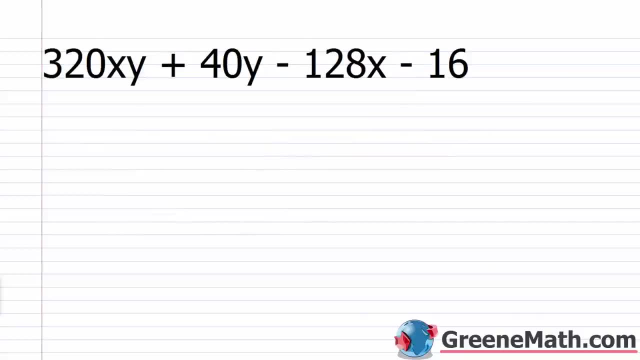 4 term polynomial back right now. sometimes you're going to have a common factor for all terms present before we begin the process. it's best to pull this out before you start because if you don't, you're going to end up with additional factoring in the end. so if I look 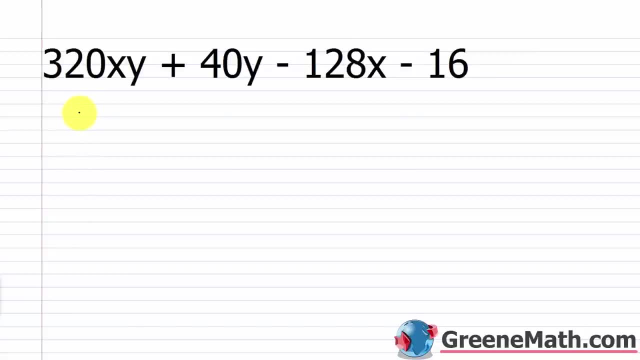 at these terms: here everything is divisible by 8. 320 divided by 8 is 40, 40 divided by 8 is 5, 128 divided by 8 is 16 and 16 divided by 8 is 2, so we can pull out this. 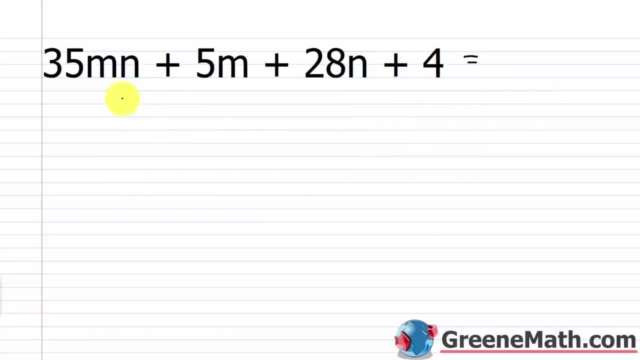 So let's go ahead and do that. So we'll put equals. Again, in this first one, I'm pulling out a 5m. 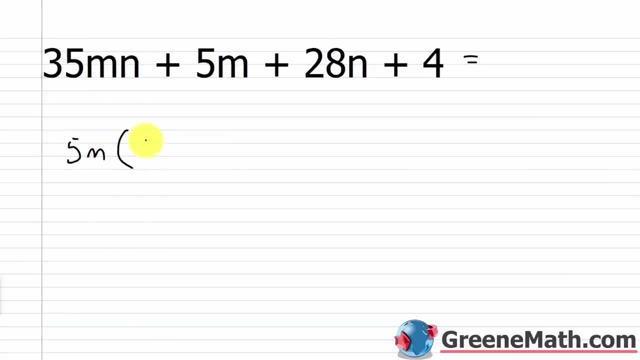 And what's left inside, 35mn divided by 5m is 7n, plus 5m over 5m is 1, plus when I'm pulling out of this group, I'm pulling out a 4. 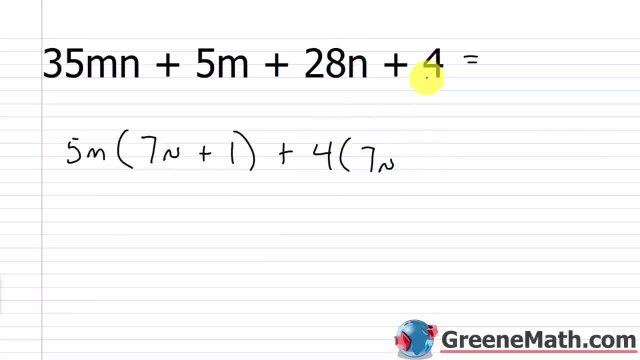 So 28n divided by 4 is 7n, and then plus 4 over 4 is 1. 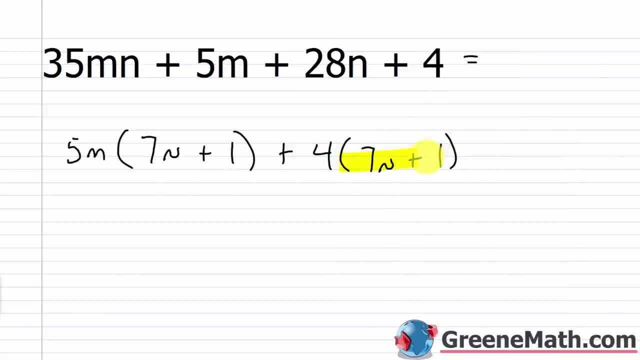 So you can see we have that common binomial factor of 7n plus 1. Okay? 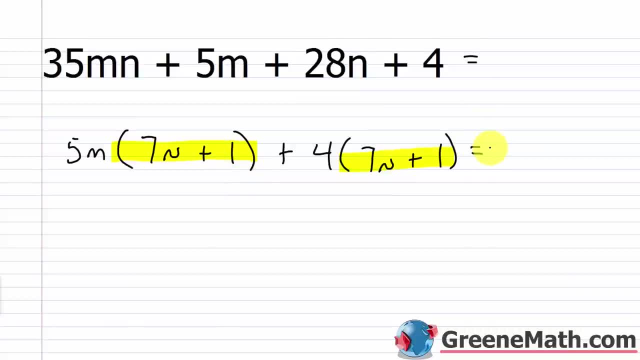 That quantity there. So if I pulled that out, I would have 7n plus 1 outside, 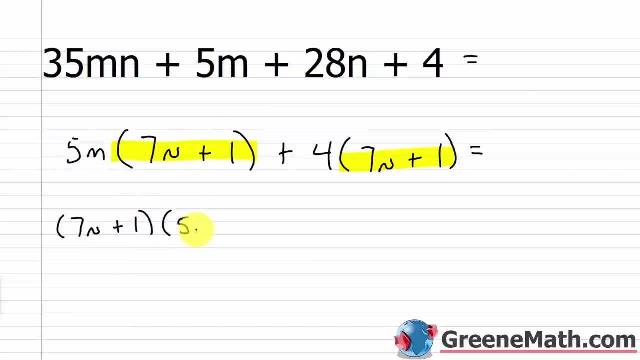 and then I would have 5m that's left here, 5m, plus from here, this is gone, so I just have a 4. So I'd have the quantity 7n plus 1 times the quantity 5m plus 4. 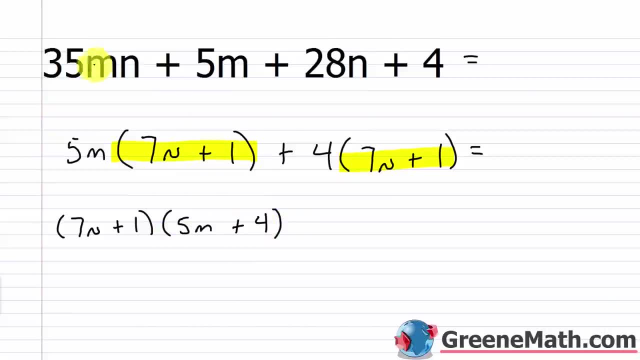 And again, if you use FOIL to check this, you're going to end up with this exact same four-term polynomial back. 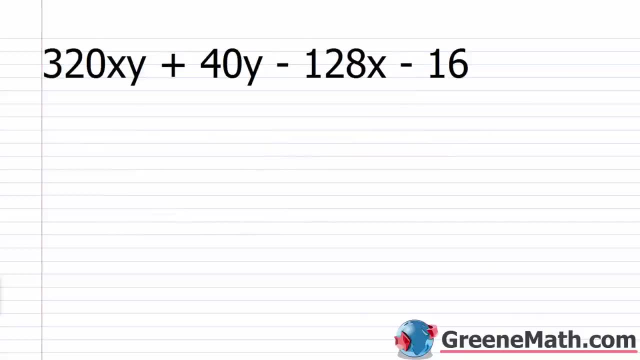 Now, sometimes you're going to have a common factor for all terms present before we begin the process. It's best to pull this out before you start because if you don't, you're going to end up with additional factoring in the end. 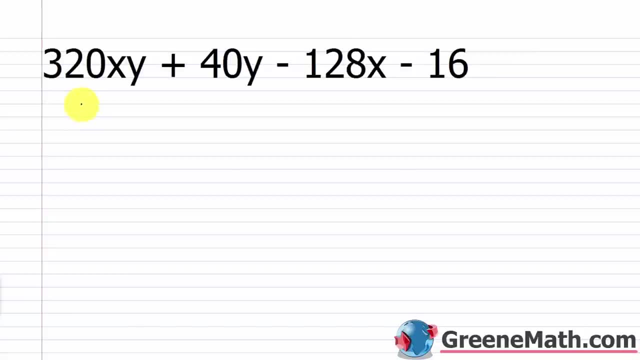 So if I look at these terms here, everything is divisible by 8. 320 divided by 8 is 40. 40 divided by 8 is 5. 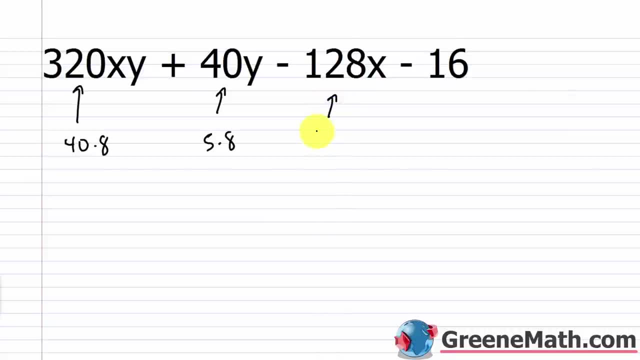 128 divided by 8. Is 16. And 16 divided by 8 is 2. 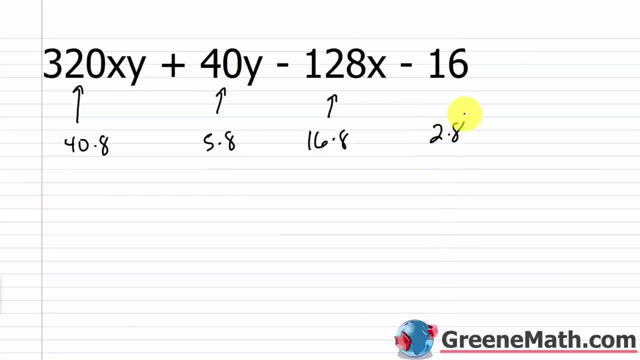 So we can pull out this common factor of 8 before we even start. So in other words, this is what this would look like. I'd put an 8 out in front, I'd put some parentheses, and then I'd say, okay, well, I have 40xy, and then plus I have 5y, and then minus I have 16x, and then minus I have 2. 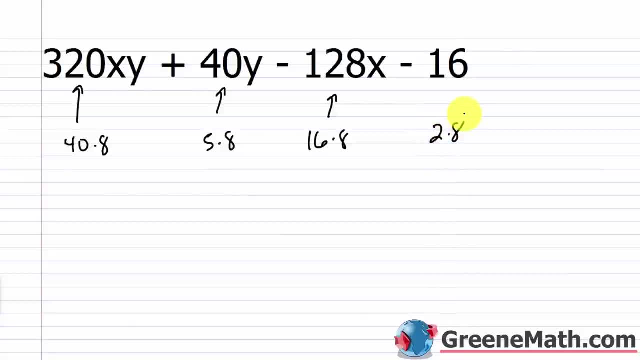 common factor of 8 before we even start. so, in other words, this is what this would look like. I'd put an 8 out in front, I'd put some parentheses, and then I'd say, ok, well, I have 40xy, and then plus, I have. 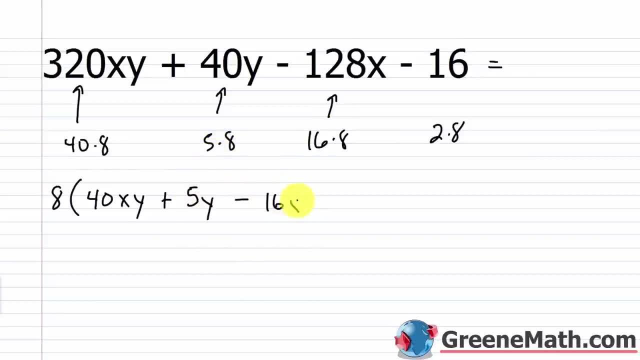 5y and then minus. I have 16x and then minus. I have 2. now, once we've done that, we just factor the inside part, just like the 8 doesn't exist. don't even worry about that, just leave it outside the parentheses. we're going to worry about that. 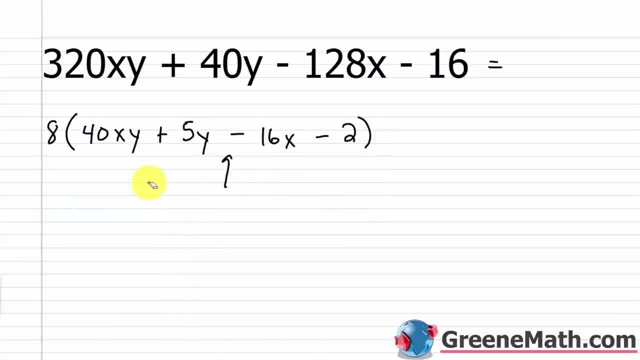 at the very, very end I'll show you what to do with it. so just work on this. so again, we can just go with the groupings that are present at first, see if they work out. so these two and these two. so 40xy and 5y. 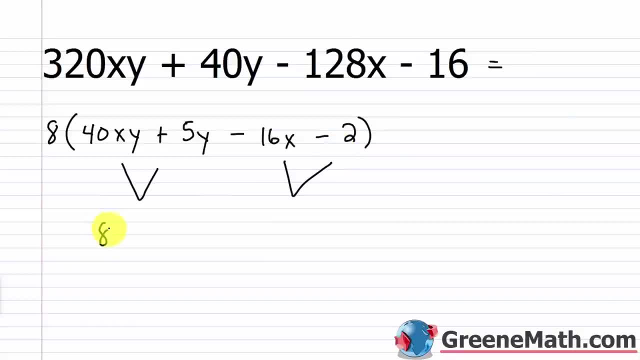 common factor of 5y, that would be 8x plus 1 and then 16x and 2. well, they're both negative, so I could pull out the negative part and I could pull out a 2. so if I pulled out a negative 2 here, 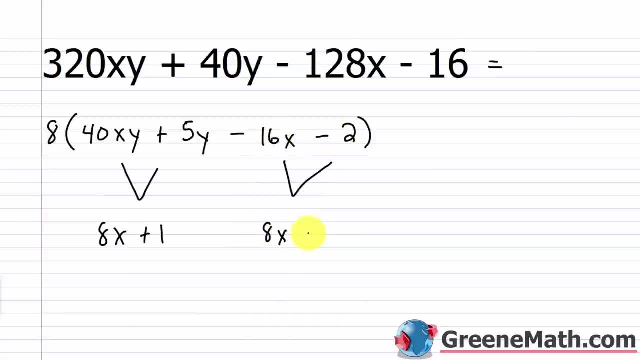 I would have 8x left if I pulled out a negative 2 here. I'd have plus 1, so it looks like that would work out. we'd have that common binomial factor and again, this is something you're going to want to do mentally. 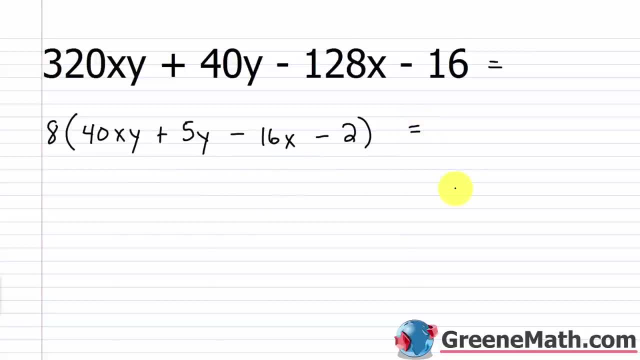 if you go through and write it all out, it's going to take you a little while, a little bit longer. so I'll rewrite the 8 and then I'm going to split this up. so 40xy plus 5y the GCF, there is 5y. 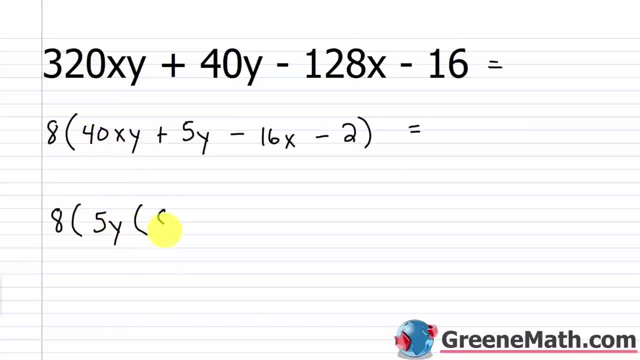 so 40xy divided by 5y would be 8x, and then plus 5y over 5y is 1. then we have this: minus 16x, minus 2. I'm going to pull out that negative part, also each negative. I'm going to pull that out. 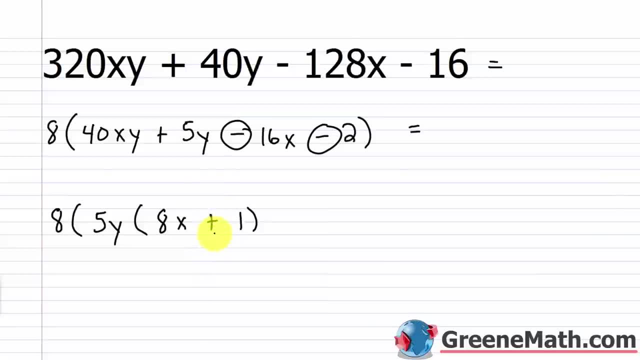 because I notice that here I have a positive. so I want that, so I can have a common binomial factor. so that's the situation where we're pulling out the negative of the GCF. so I'm going to pull out negative 2 and let me just put plus negative 2. 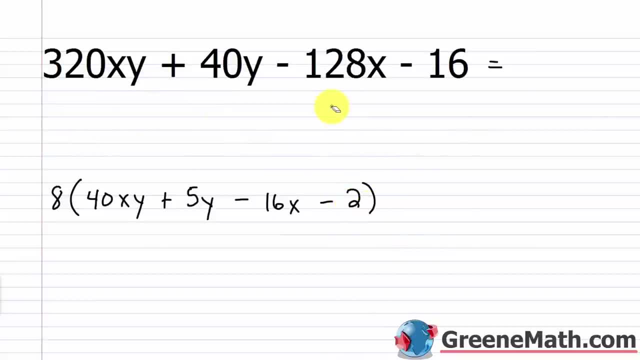 Now, once we've done that, we just factor the inside part, just like the 8 doesn't exist. Don't even worry about that. Just leave it outside the parentheses. 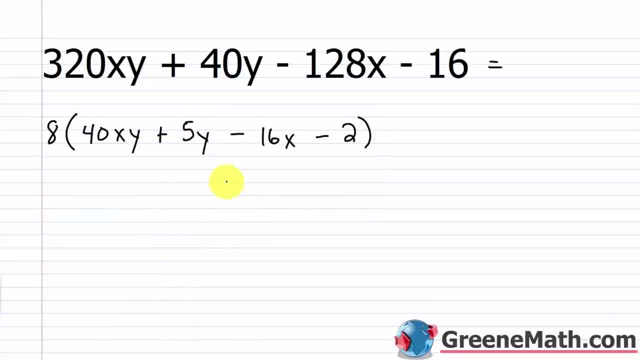 We're going to worry about that at the very, very end. I'll show you what to do with it. So just work on this. 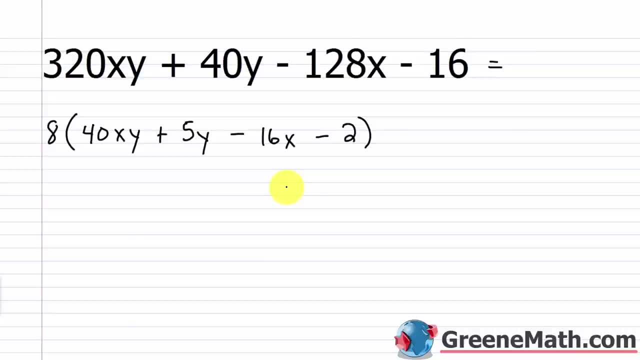 So again, we could just go with the groupings that are present at first, see if they work out. 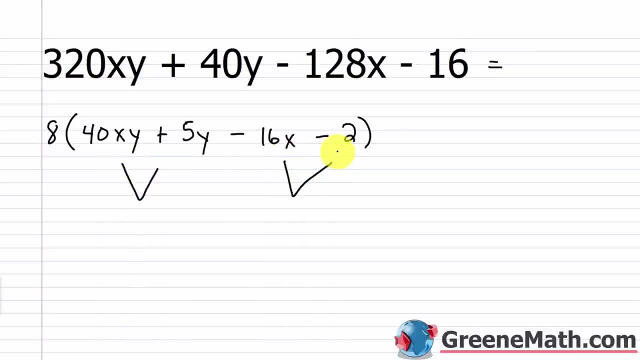 So these two and these two. So 40xy and 5y, common factor of 5y, 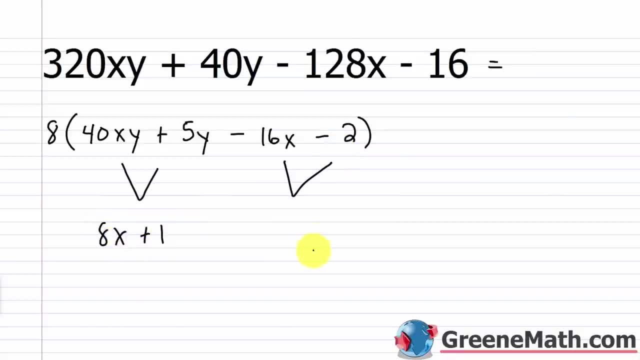 that would be 8x plus 1, and then 16x and 2. Well, they're both negative, so I could pull out the negative part, and I could pull out a 2. So if I pulled out a negative 2 here, I would have 8x left. 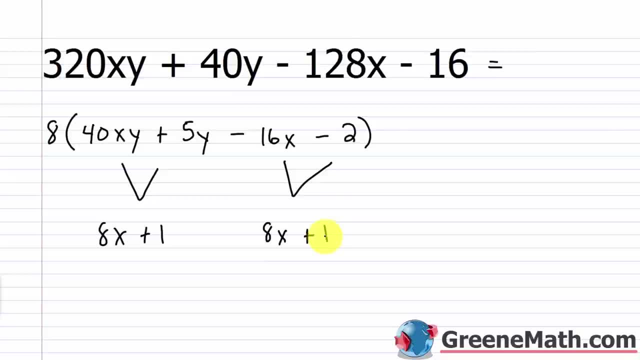 If I pulled out a negative 2 here, I'd have plus 1. So it looks like that would work out. We'd have that common binomial factor. 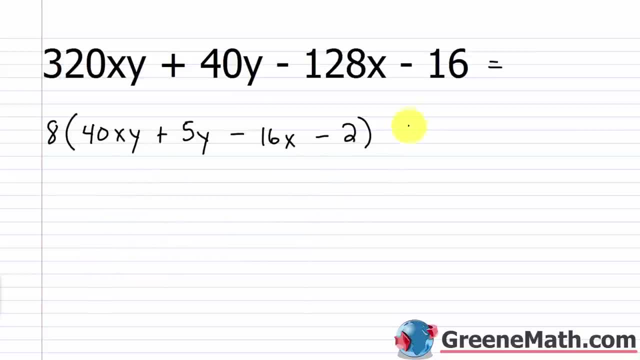 Again, this is something you're going to want to do mentally. If you go through and write it all out, it's going to take you a little bit longer. 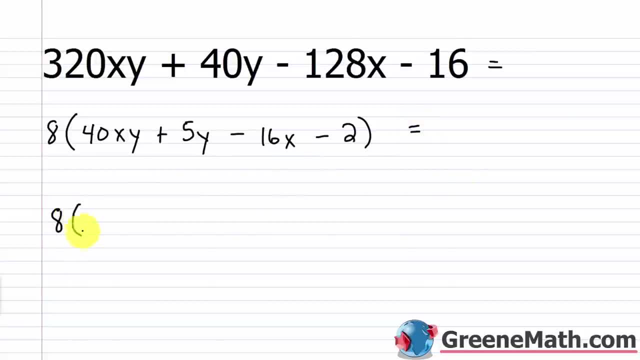 So I'll rewrite the 8, and then I'm going to split this up. So 40xy plus 5y, the GCF there is 5y. 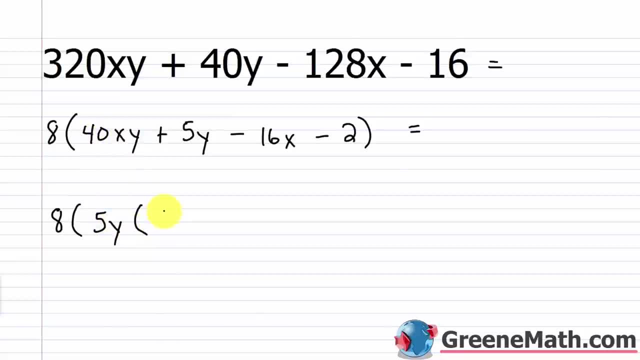 So 40xy divided by 5y would be 8x, and then plus 5y over 5y is 1. 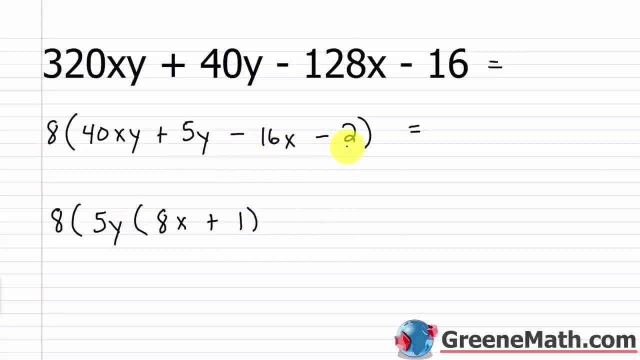 Then we have this minus 16x minus 2. I'm going to pull out that negative part also. So each negative, I'm going to pull that out, because I notice that here I have a positive. So I want that so I can have a common binomial factor. So that's the situation where we're pulling out the negative of the GCF. 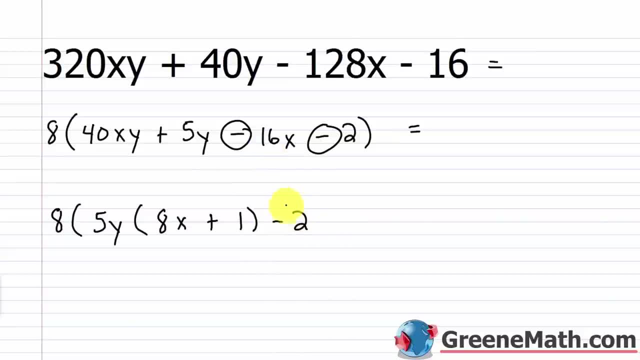 So I'm going to pull out negative 2, and let me just put plus negative 2, because that always looks a little better to me. 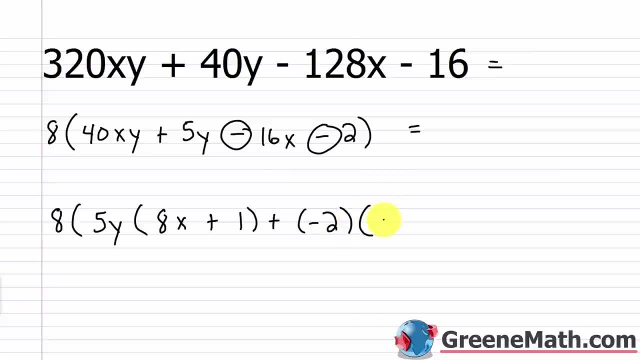 inside of here, 16x over 2 would be 8x. 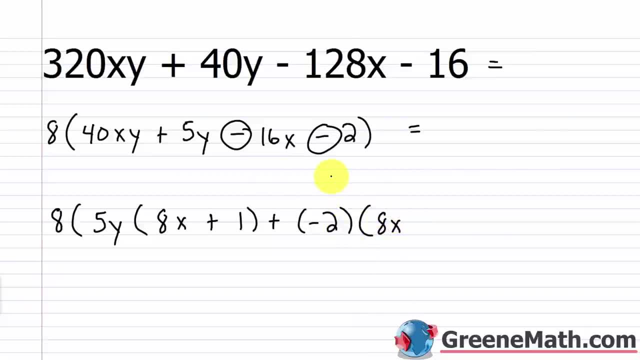 And again, I've already taken care of the signs, so I'm just thinking about the numbers as if they were positive. 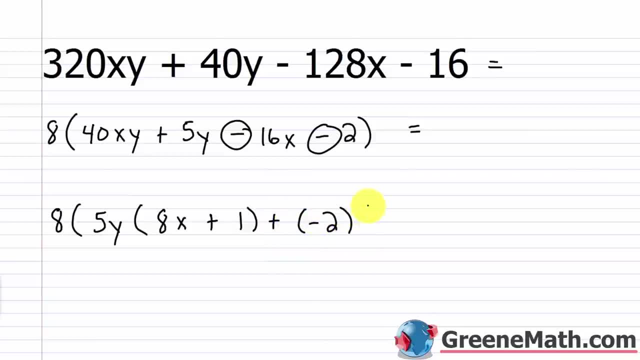 because that always looks a little better. so plus negative 2 times inside of here, 16x over 2 would be 8x, and again, I've already taken care of the signs, so I'm just thinking about the numbers as if they were positive. and then 2 over 2 is 1. 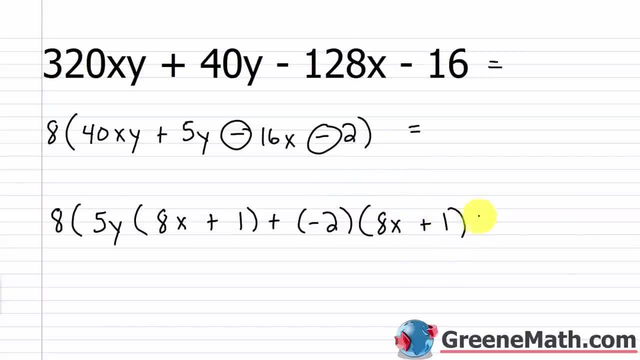 so plus 1. ok, so let me kind of close the parentheses here and again you can see you have a common binomial factor: 8x plus 1. 8x plus 1, so that's what we're going to factor out. so I have the 8 out in front. 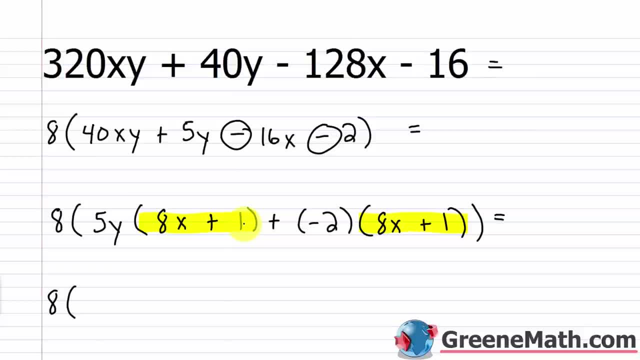 that's going to stay there, and then times this common binomial factor, that's 8x plus 1, and then times what's going to be left inside here, well, what I'm going to have if 8x plus 1 was gone. so if I just line that out, 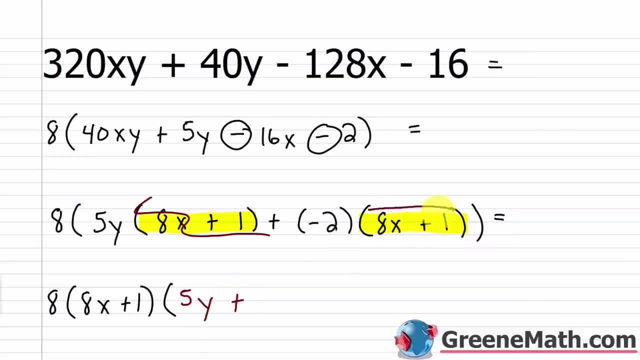 I'd have a 5y, then plus. if 8x plus 1 was gone, I'd have a negative 2. so you can put plus negative 2 or you can just put minus 2, it doesn't really matter- and close the parentheses there. 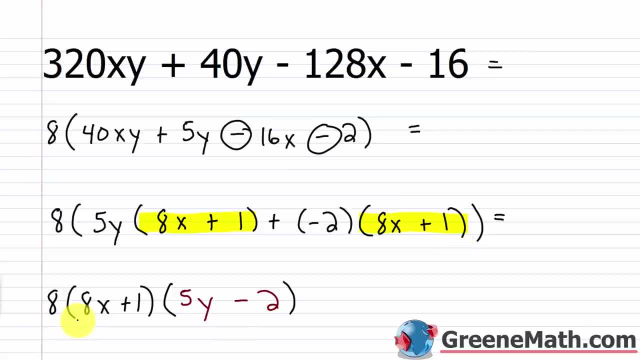 and we have our answer. we have 8 times the quantity 8x plus 1 times the quantity 5y minus 2. now this is factored completely. I'm going to show you what would happen if you didn't do this step when you begun. 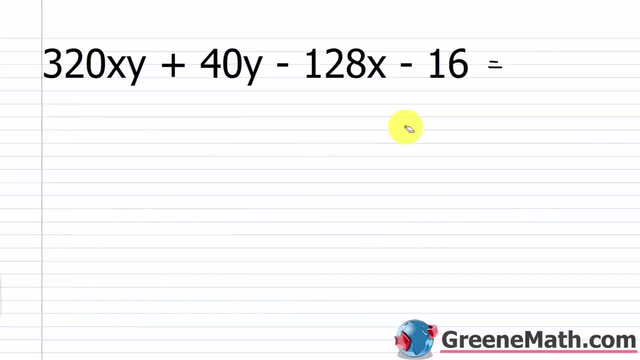 you would have had something that had additional factoring that needed to be done. so if I look at these two groups here, what can I pull out? well, I can pull out a 40y. so I pull out a 40y and I would have what? 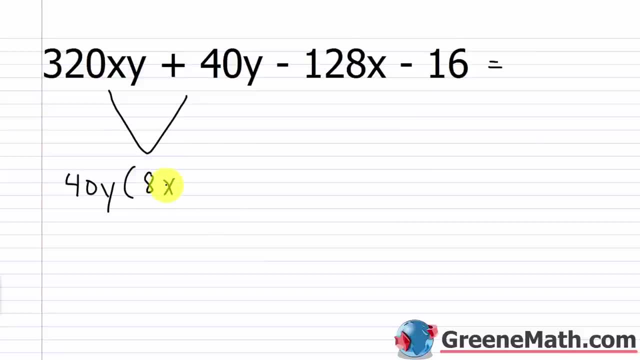 I would have 8 x plus 1. then over here I could pull out negative 16 and inside I'd have again 8x plus 1. so if I factored the common binomial factor of 8x plus 1 out, I'd have 8x plus 1. 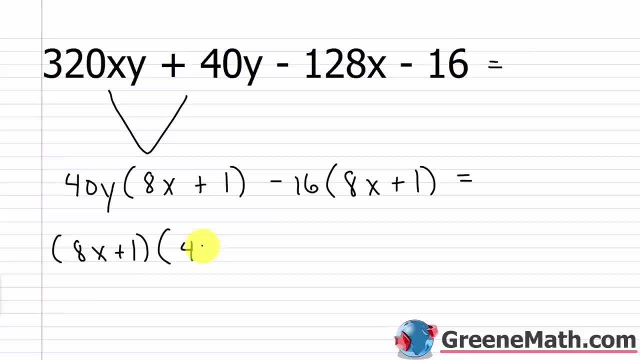 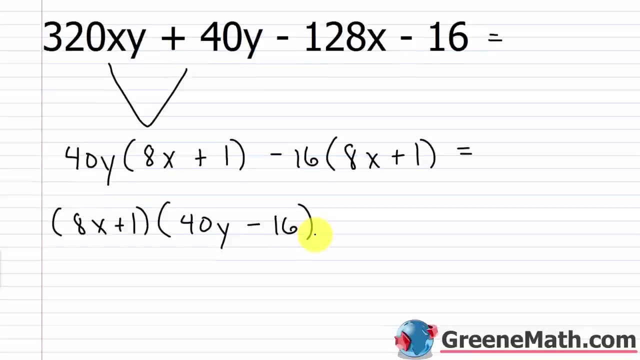 times what's left inside would be 40y. this would go away, and then you'd just have the negative 16, because this would be gone. and if you look at the 8x plus 1, that's fine. there's nothing else I can take out of there. 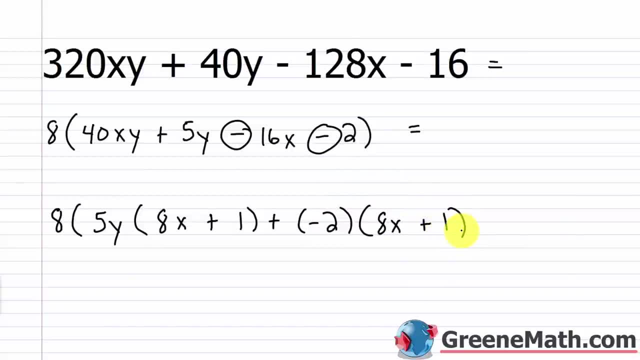 And then 2 over 2 is 1, so plus 1. 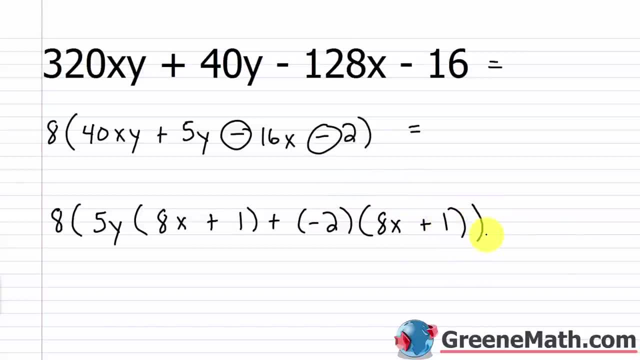 Okay, so let me kind of close the parentheses here. And again, you can see you have a common binomial factor. 8x plus 1, 8x plus 1. So that's what we're going to factor out. So I have the 8 out in front. That's going to stay there. And then times this common binomial factor, that's 8x plus 1. And then times, what's going to be left inside here? Well, what I'm going to have, if 8x plus 1 was gone, so if I just line that out, I'd have a 5y. 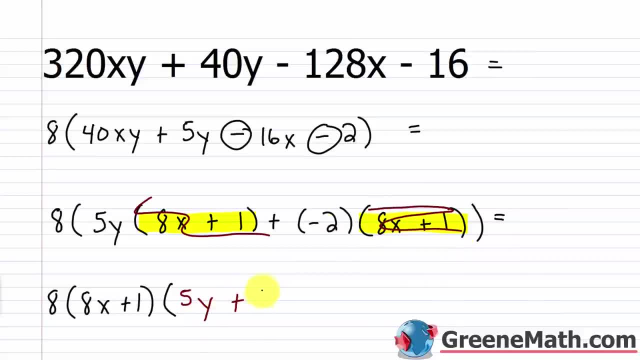 Then plus. If 8x plus 1 was gone, I'd have a negative 2. 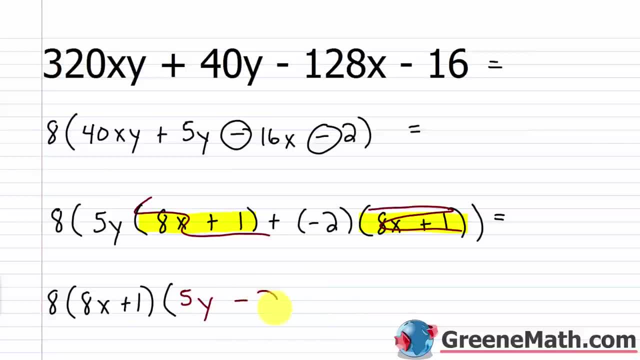 So you can put plus negative 2, or you can just put minus 2. It doesn't really matter. 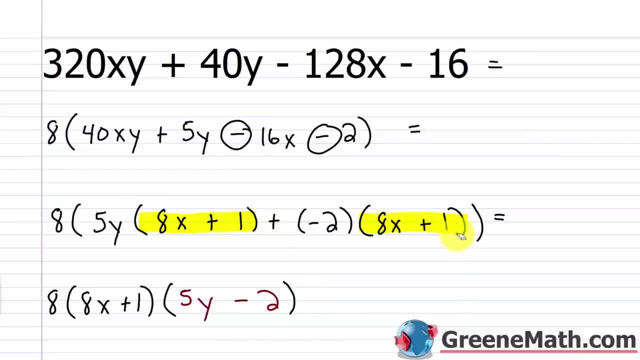 And close the parentheses there. And we have our answer. 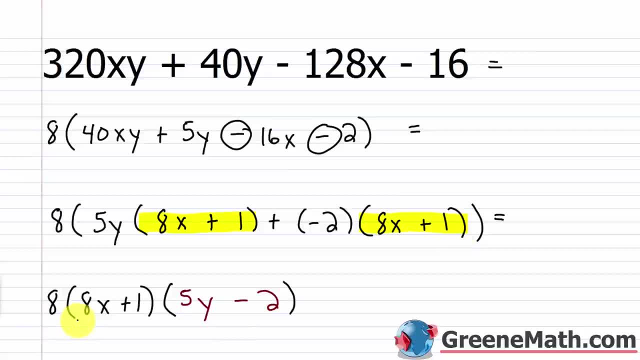 We have 8 times the quantity 8x plus 1 times the quantity 5y minus 2. 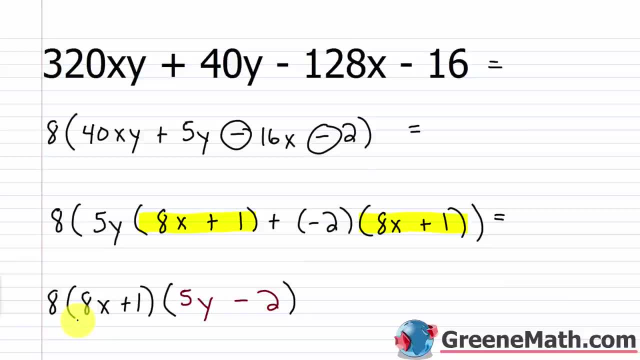 Now this is factored completely. I'm going to show you what would happen if you didn't do this step when you begun. 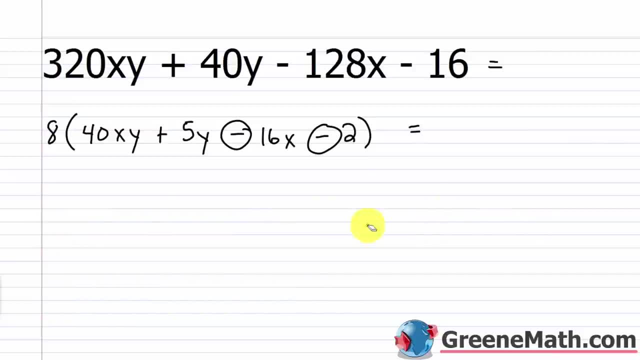 You would have had something that had additional factoring that needed to be done. 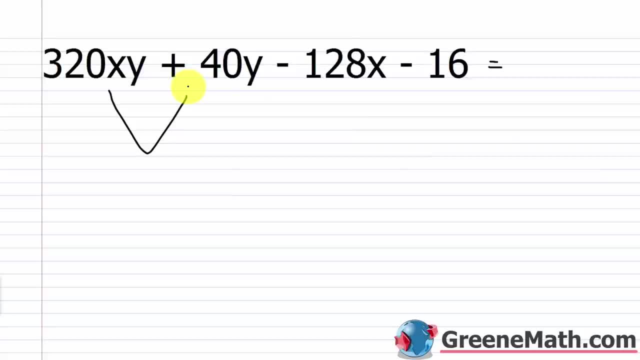 So if I look at these two groups here, what can I pull out? Well, I can pull out a 40y. So I pull out a 40y, and I would have what? 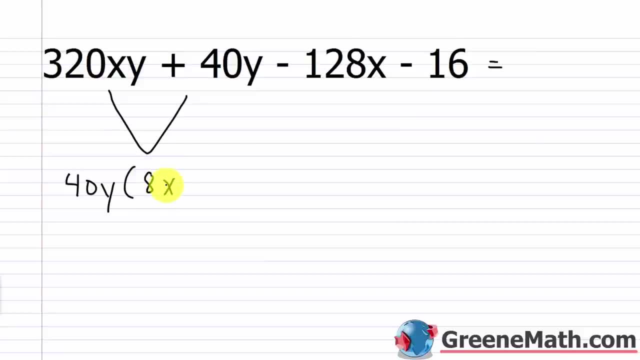 I would have 8x plus 1. Then over here, I could pull out a negative 16. And inside I'd have, again, 8x plus 1. 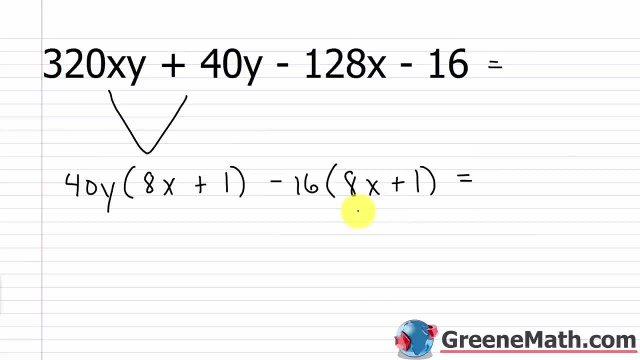 So if I factored the common binomial factor of 8x plus 1 out, I'd have 8x plus 1 times what's left inside would be 40y. 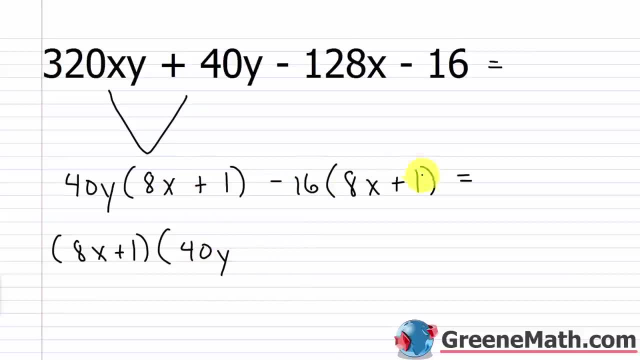 This would go away. And then you just have the negative 16, right? Because this would be gone. So minus 16. And if you look at the 8x plus 1, that's fine. 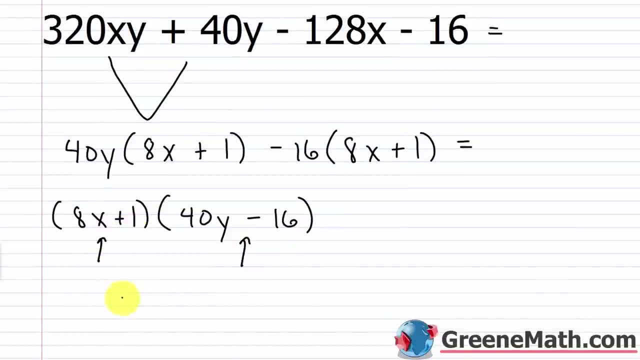 There's nothing else I can take out of there. But if I look at this right here, 40y minus 16, there's something I can pull out of there. 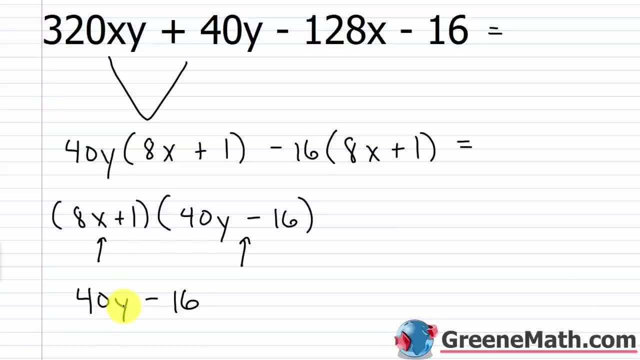 8 is common to both. So if I report my answer like this on my test, my teacher is going to go over here and she's going to put wrong. 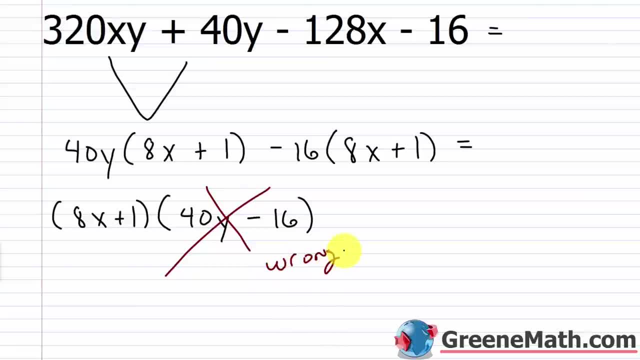 Because I didn't factor completely. There was something else I could have pulled out. 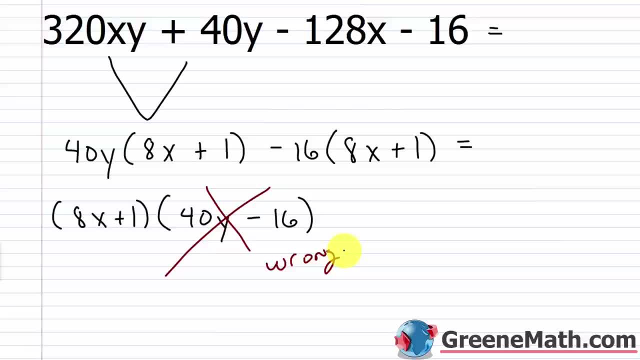 You've got to keep that in mind when you're doing a test or homework. You might have factored, but you didn't factor completely, 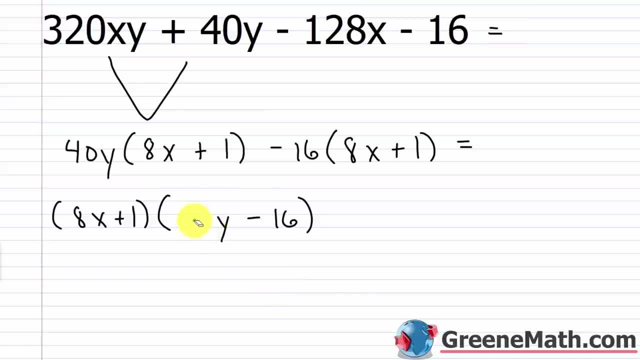 If I pull out an 8 from here, 8 divided by 8 is 5. So this should be 5y. So this 8 is going to go out here. If I pull out an 8 from here, this would be 2. 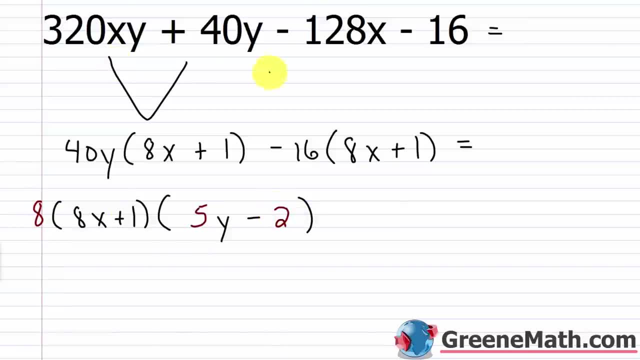 So this is how we got our original answer. But again, I pulled out the 8 to begin with. So I didn't have to go through that additional step in the end. 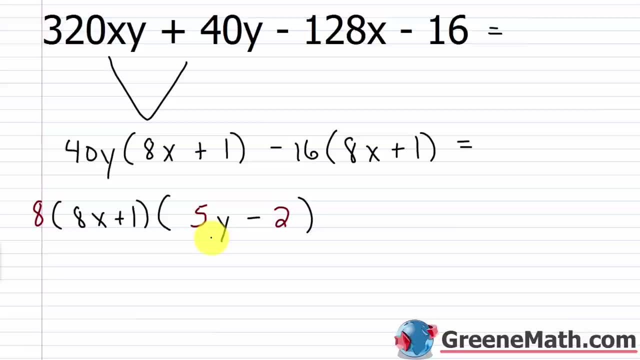 So if you don't want to pull it out, and you want to do additional factoring in the end, that's fine. But you have to look for it. 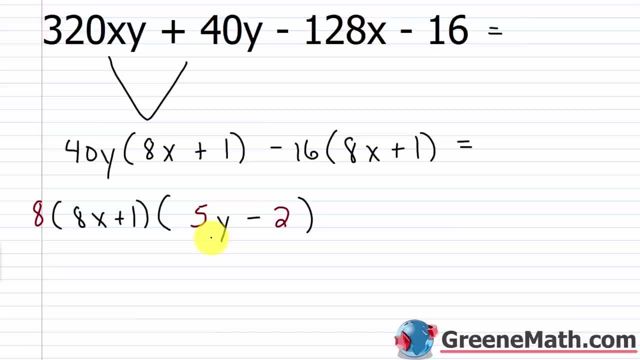 You have to always be looking for additional factoring that needs to be done. 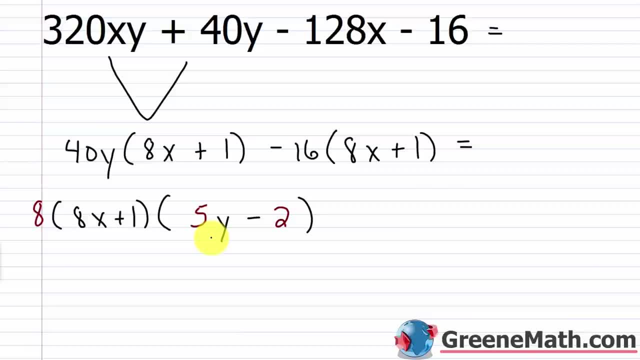 Because that's the quickest way to get either a wrong answer, or at minimum, points off on your test or homework by not factoring completely. 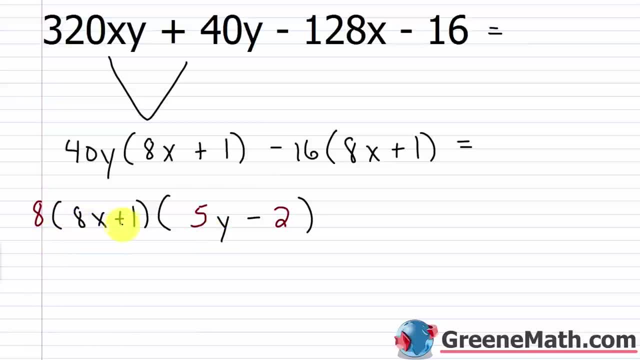 Alright, so the answer here is 8 times the quantity, 8x plus 1, times the quantity, 5y minus 2. 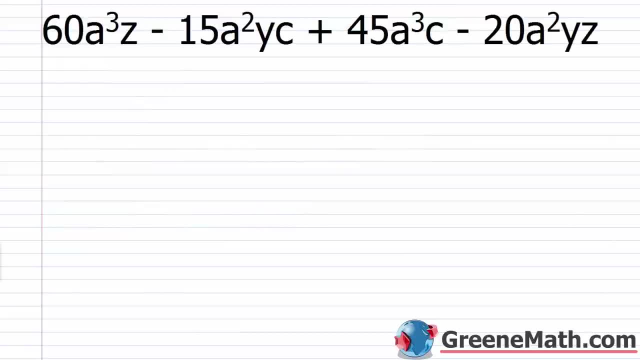 Alright, let's take a look at another one. We have 60a cubed z, 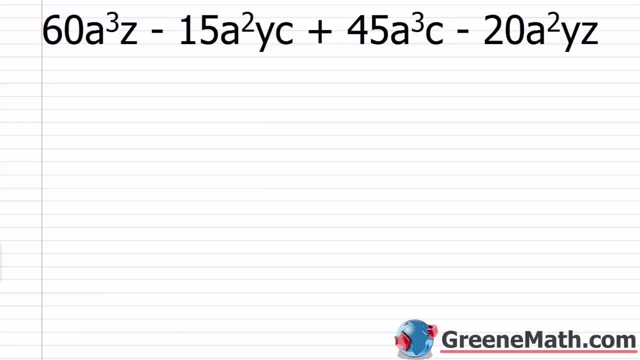 minus 15a squared yc, plus 45a cubed c, 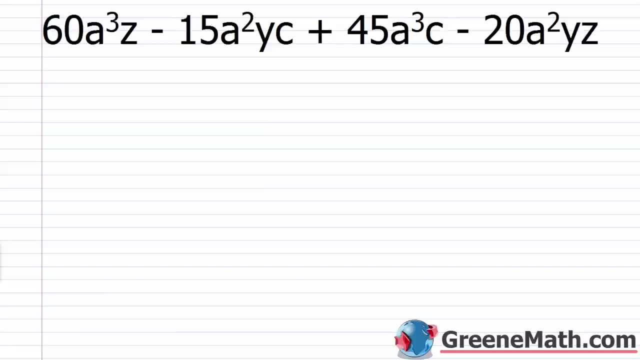 minus 20a squared yz. 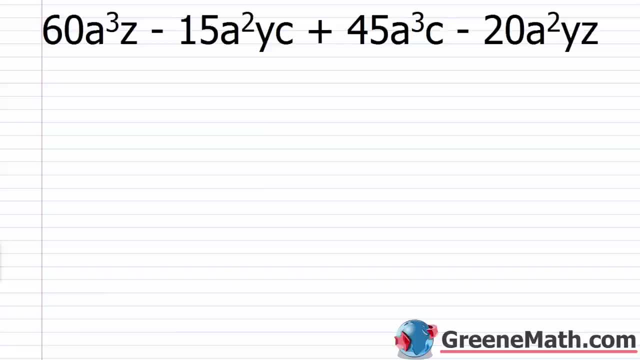 So again, if I look here carefully, I notice that 5 is common to everything before I even start. 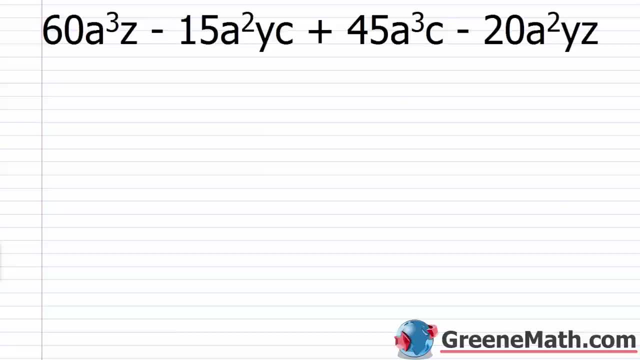 And also, a squared is common to everything before I start. 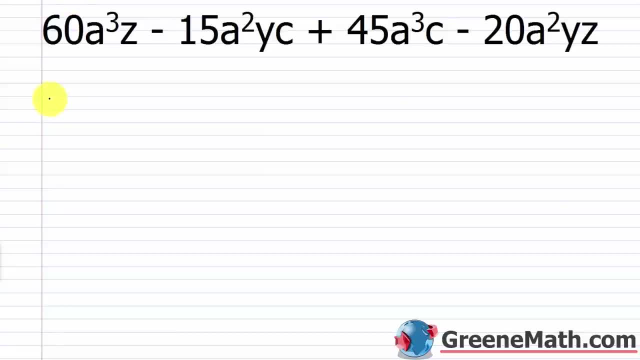 So before I do anything, I can pull that out. So I can pull out a 5a squared, and rewrite this whole thing here. 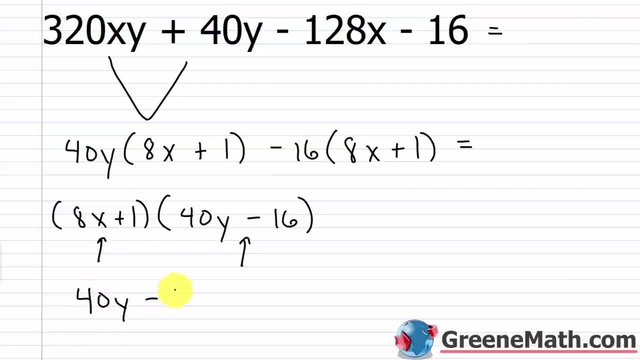 but if I look at this right here, if I look at 40y minus 16, there's something I can pull out of there. 8 is common to both. so if I report my answer like this on my test, my teacher is going to go over here. 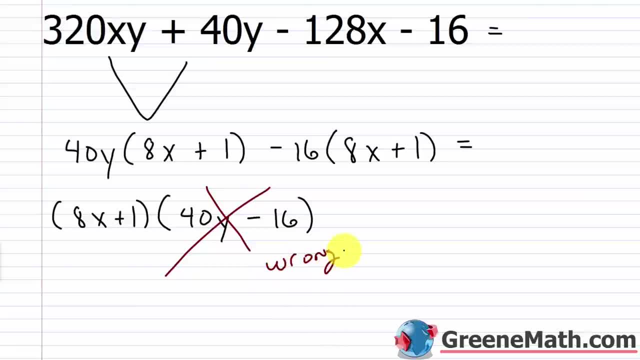 and she's going to put wrong because I didn't factor completely. there was something else I could have pulled out. you've got to keep that in mind when you're doing a test or homework. you might have factored, but you didn't factor completely, so the answer is wrong. 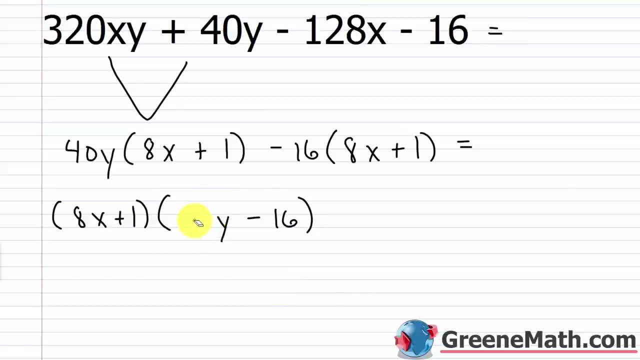 if I pull out an 8 from here, 40 divided by 8 is 5, so this should be 5y. if I pull out an 8 from here, this would be 2. so this is how we got our original answer, but again I pulled out the 8. 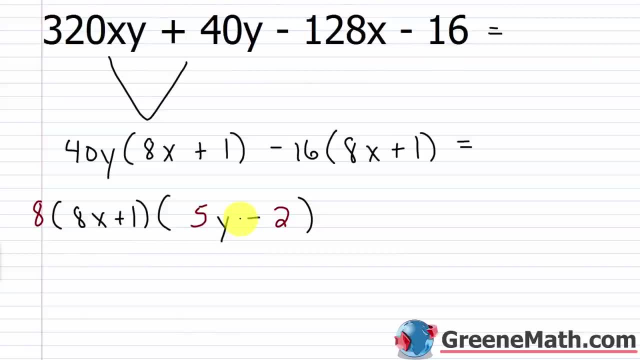 to begin with. so I didn't have to go through that additional step in the end. so if you don't want to pull it out and you want to do additional factoring in the end, that's fine, but you have to look for it. you have to always be looking. 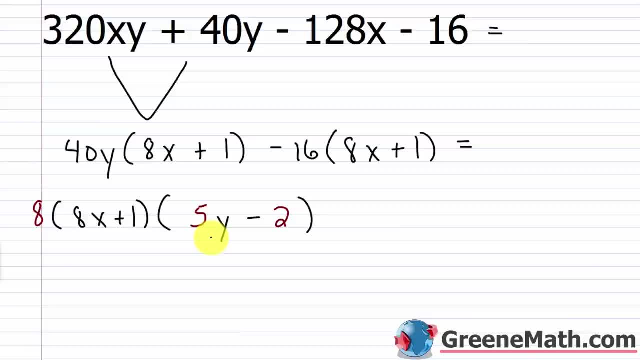 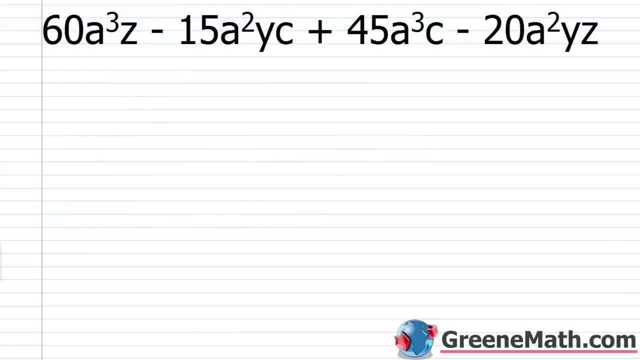 for additional factoring. that needs to be done because that's the quickest way to get either a wrong answer or, at minimum, points off on your test or homework by not factoring completely. so the answer here is 8 times the quantity. times the quantity. alright, let's take a look at another one. 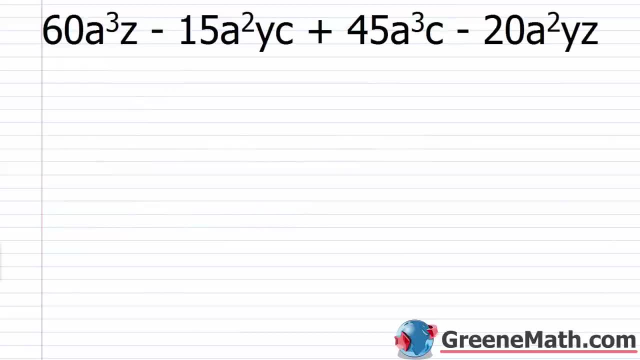 we have 60a cubed z minus 15a squared yc, plus 45a cubed c minus 20a squared yz. so again, if I look here carefully, I notice that 5 is common to everything, before I even start, and also a squared. 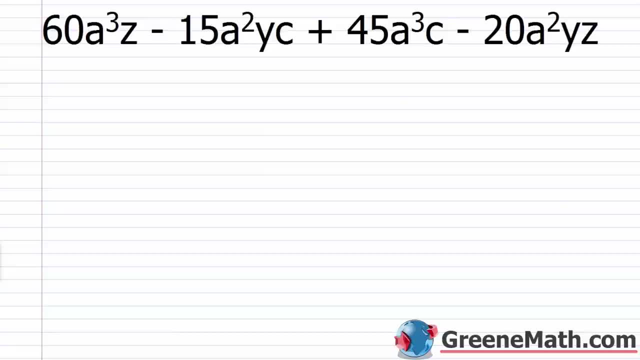 is common to everything. before I start, so before I do anything, I can pull that out. so I can pull out a 5a squared and rewrite this whole thing here: 60 divided by 5 is 12. a cubed over a squared is a, so az. 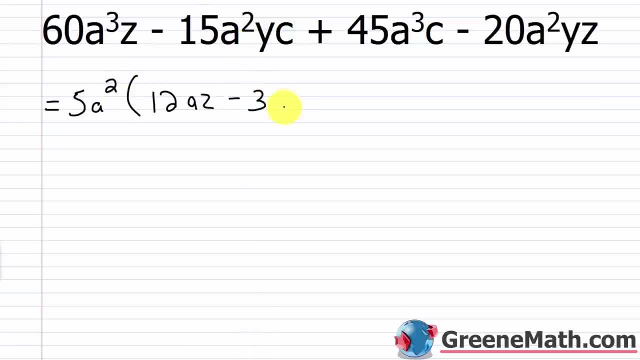 minus 15 divided by 5 is 3. a squared over a squared is 1, so this should be yc plus 45 divided by 5 is 9. a cubed over a squared is a, and then times c, and then minus 20 over 5 is 4. 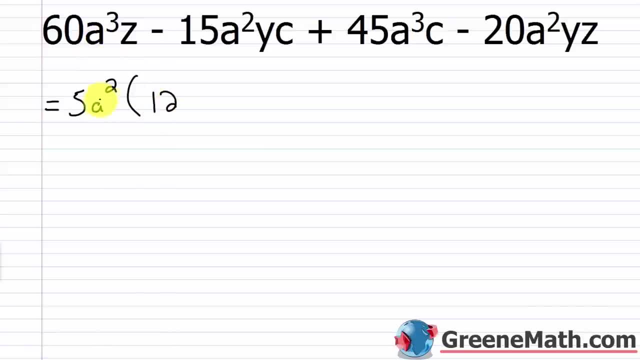 60 divided by 5 is 12, a cubed over a squared is a, so az, minus 15 divided by 5 is 3, a squared over a squared is 1, so this should be yc, plus 45 divided by 5 is 9, 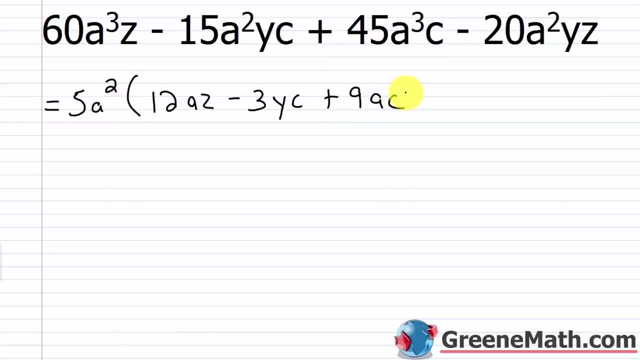 a cubed over a squared is a, and then times c, and then minus 20 over 5 is 4, 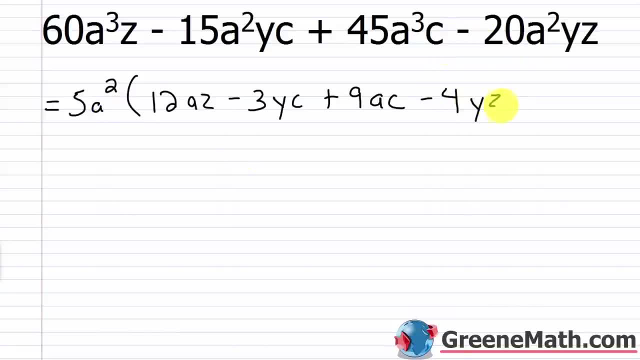 a squared over a squared is 1, and then yz. 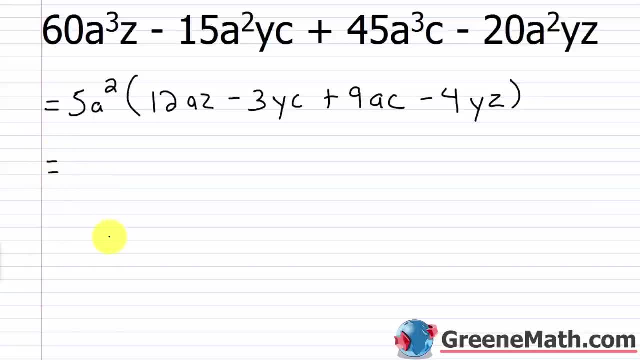 Okay, so now, I just go through and factor by grouping just as I normally would. 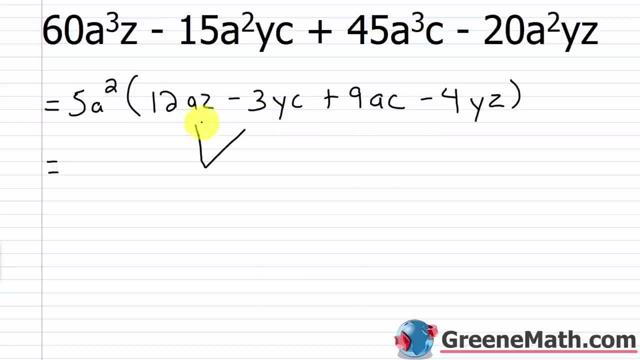 So again, I'm going to look at what's already in order, so these two as a group, and these two as a group. Would that work out? 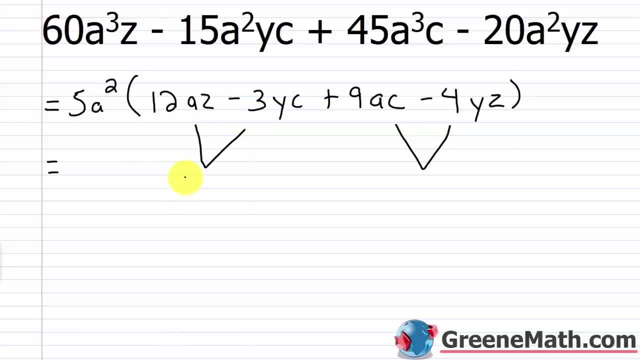 I have 12 and I have 3, so the greatest common factor there would be 3. I have az and I have yc, so nothing I can pull out for the variables. So if I did that, I would end up with what? 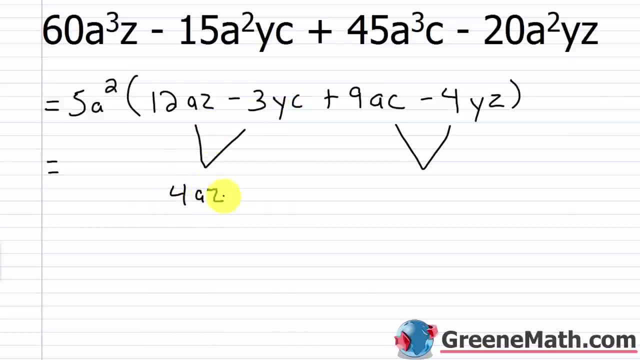 I would end up with a 4az, and if I pulled out a 3 there, that would be minus yc, and so here, I would end up with what? 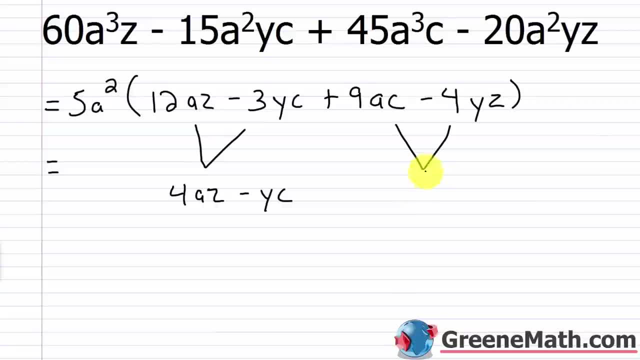 9 and 4, nothing I can really do there other than 1, ac and yz, nothing I can really do there. So 1 is the only thing I could pull out, so you'd have 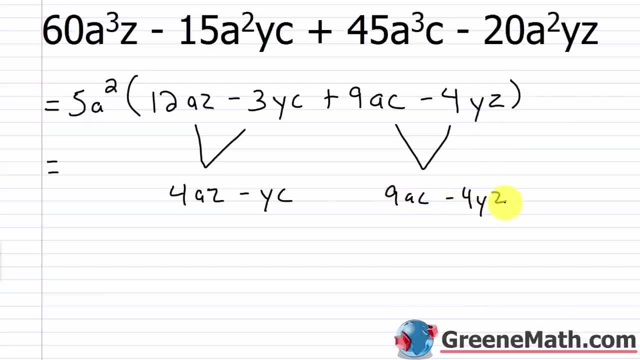 9ac minus 4yz, so we would not yield a common binomial factor here. 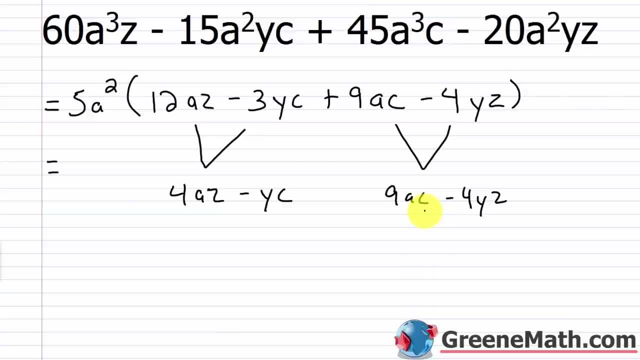 So we would have to reorder our terms to get a common binomial factor. 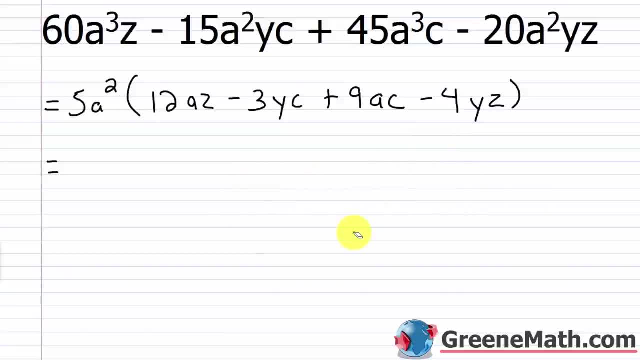 So let's go ahead and try a different grouping. So I noticed that this has a z, and this has a z, this has a 4, this has a 12, 12 is 4 times 3. 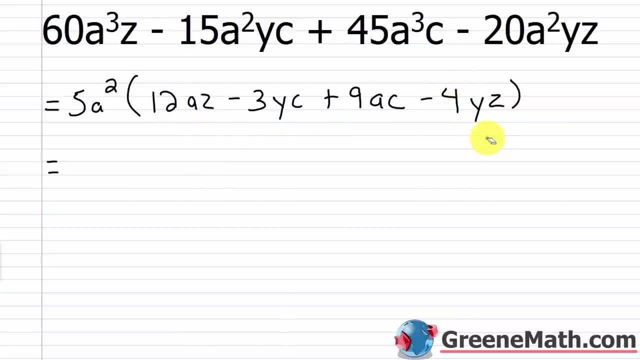 So let's try writing, let's try writing 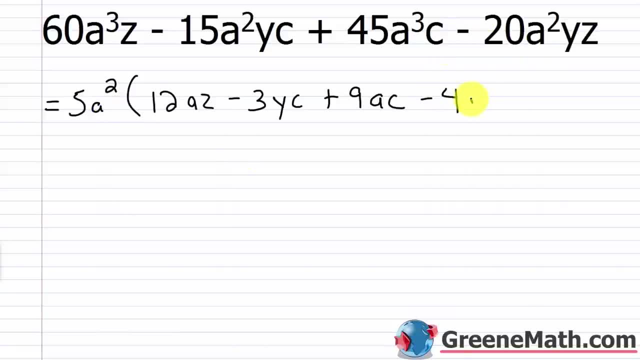 a squared over a squared is 1 and then yz. ok, so now I just go through and factor by grouping, just as I normally would. so again, I'm going to look at what's already in order. so these two as a group and these two as a group. 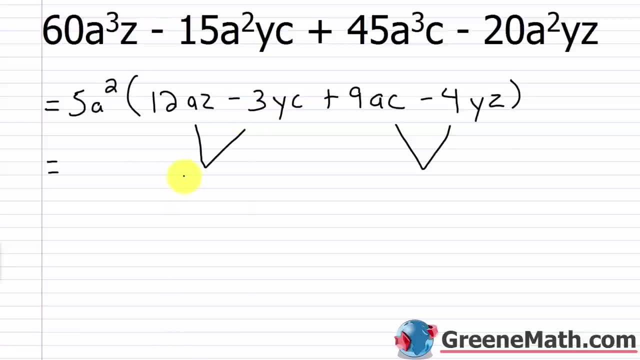 would that work out? I have 12 and I have 3, so the greatest common factor there would be 3. I have az and I have yc as variables. so if I did that, I would end up with what I would end up with: a 4az. 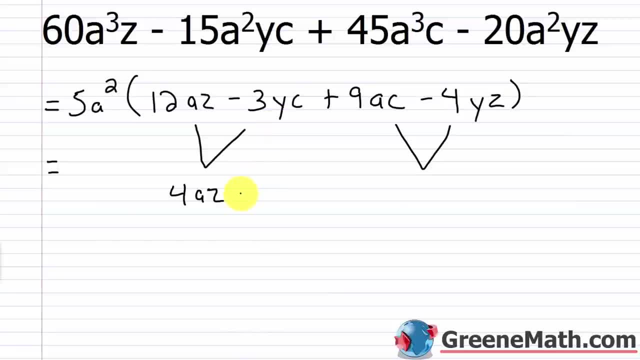 and if I pulled out a 3 there it would be minus yc, and so here I would end up with what? 9, and 4. nothing I can really do there other than 1, ac and yz. nothing I can really do there, so 1 is the only. 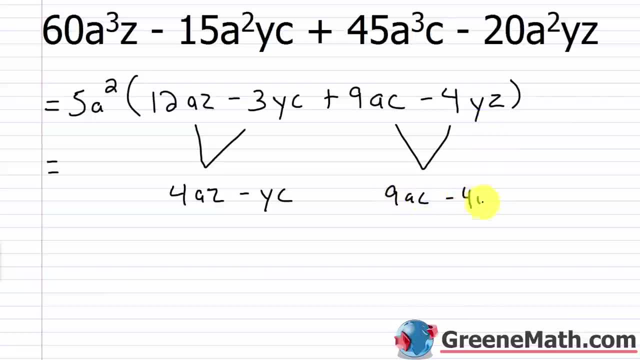 thing I could pull out, so you'd have 9ac minus 4yz. so we would not yield a common binomial factor here, so we would have to reorder our terms to get a common binomial factor. so let's go ahead and try a different grouping. 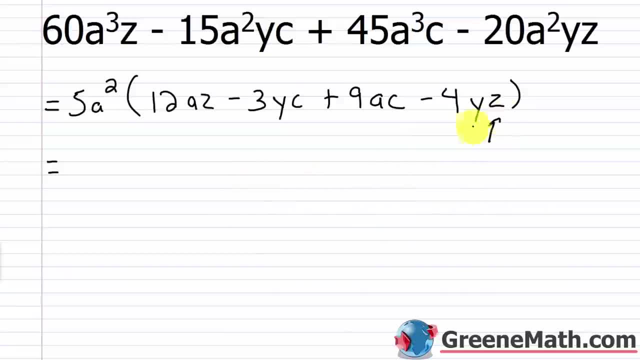 so I noticed that this has a z and this has a z. this has a 4, this has a 12. 12 is 4 times 3. so let's try writing. let's try writing 5a squared times the quantity 12az. then I'm going to put minus 4yz. 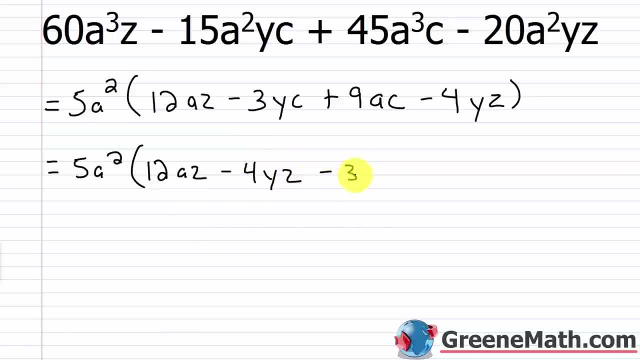 so this could be a group, and then minus 3yc, plus 9ac. so now let's look at the way it's set up here. so- and this one's a little complex, so I'm going to actually have to write it out- so I'm going to put 5a squared. 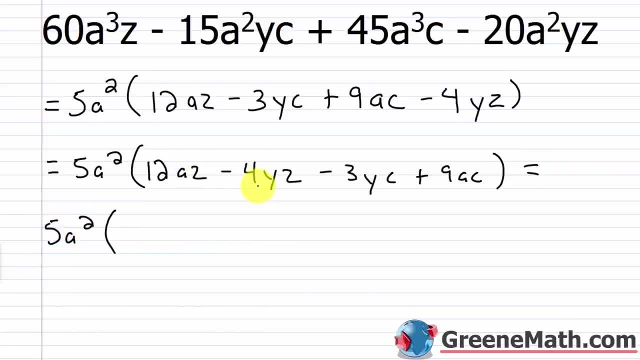 times what's common here? I have a 4 and a z right, so I could pull out a negative 4z also, but let's see if we need to do that. let's just start out with positive 4z. so what's going to be left inside the parentheses? 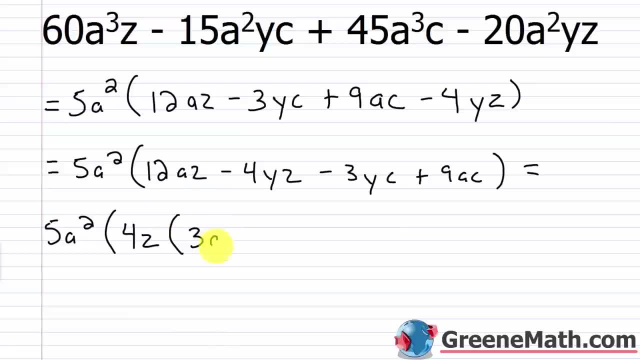 12 divided by 4 is 3. z over z is 1, so just 3a. then minus 4 over 4 is 1. z over z is 1, so just y. now I have this negative out in front. with these two, it's a negative 3yc. 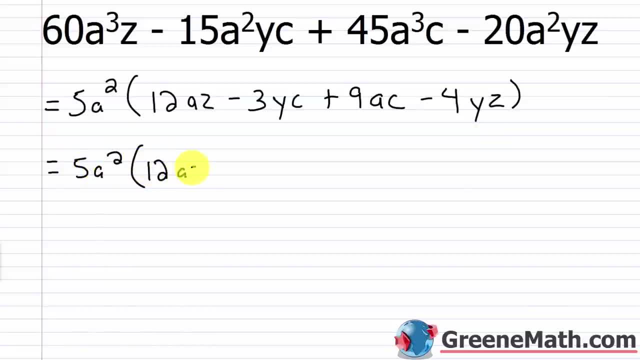 5a squared times the quantity, 12az, then I'm going to put minus 4yz, so this could be a group, 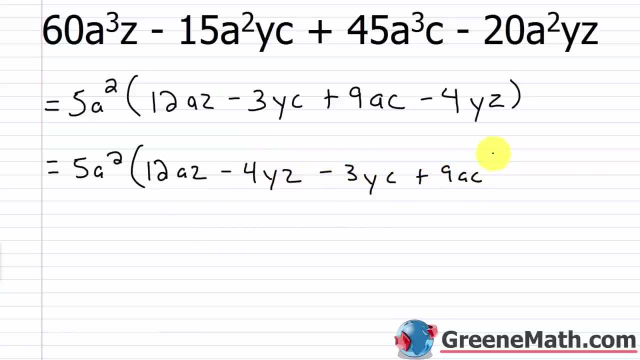 and then minus 3yc plus 9ac. 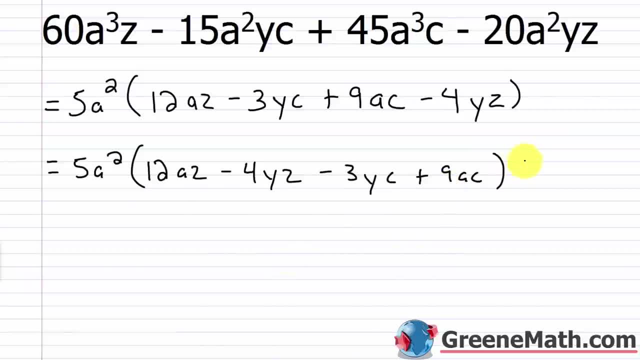 So now let's look at the way it's set up here. So, and this one's a little complex, so I'm going to actually have to write it out. 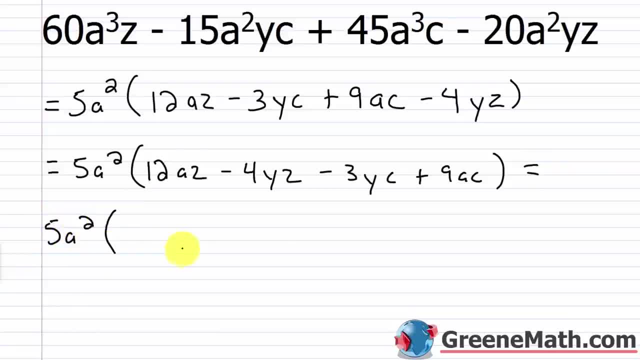 So I'm going to put 5a squared times, what's common here? 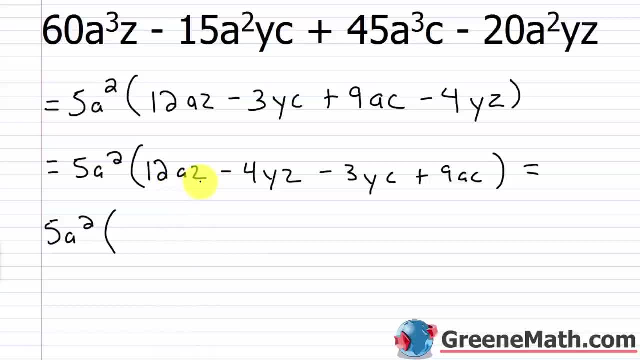 I have a 4 and a z. So I could pull out a negative 4z also, but let's see if we need to do that. 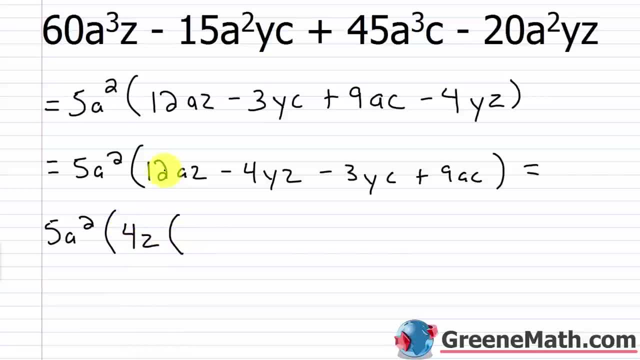 Let's just start out with positive 4z. So what's going to be left inside the parentheses, 12 divided by 4 is 3, z over z is 1, so just 3a. Then minus, 4 over 4 is 1, z over z is 1, 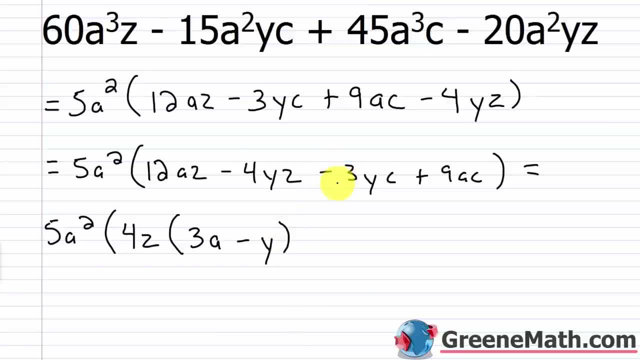 so just y. Now I have this negative out in front. With these two, 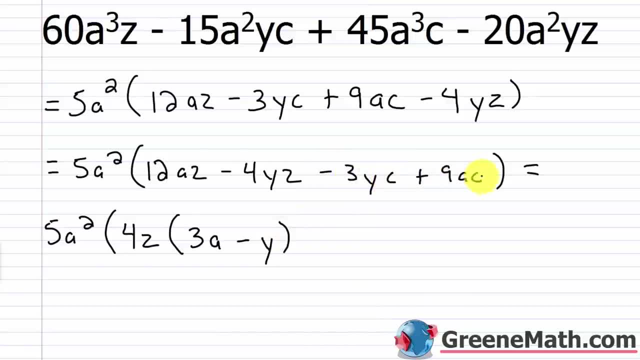 it's a negative 3yc, and it's a positive 9ac. So I can start by just factoring out a negative 3c. 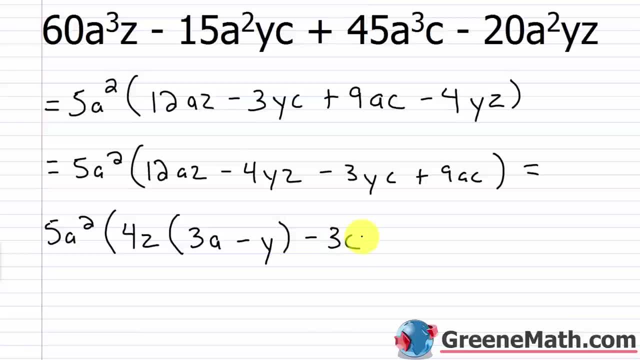 So I'm going to put negative 3c out in front, and I like to put plus negative. That's just me. 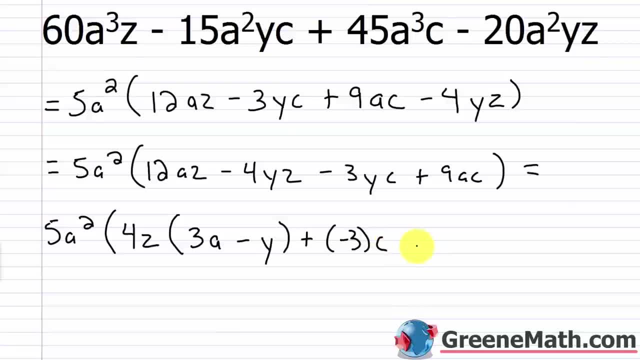 So I'm going to put plus negative 3c. And then inside, if I pulled out a negative 3c, I would just have a y. 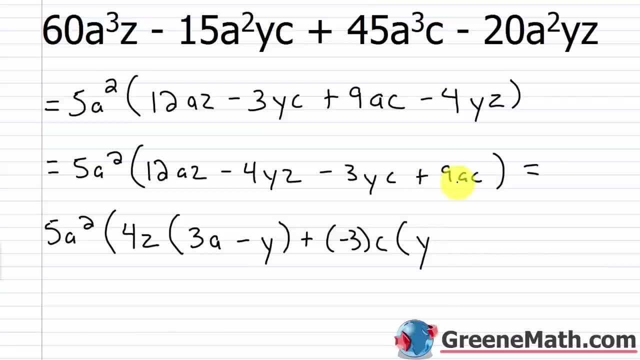 And then if I pulled out a negative 3c, all that's going to happen here is the sign's going to change. So this would be negative, and then you'd have a 3, right? 9 over 3 is 3. And then the c would cancel, so you just have an a. 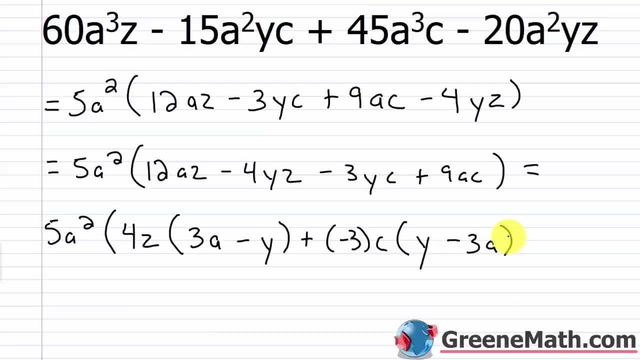 Now, I don't have a common binomial factor yet, but we're close, right? We have a y and a y, and we have a 3a and a 3a. 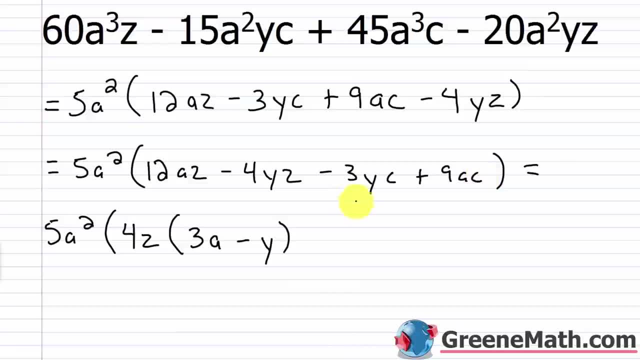 and it's a positive 9ac. so I can start by just factoring out a negative 3c. so I'm going to put negative 3c out in front and I like to put plus negative. that's just me, so I'm going to put. 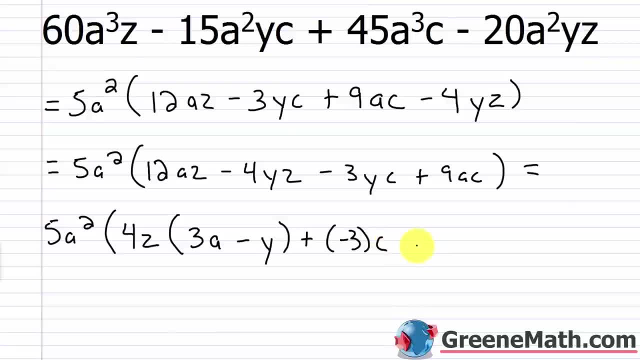 plus negative 3c and then inside. if I pulled out a negative 3c, I would just have a y, and then, if I pulled out a negative 3c, all that's going to happen here is the sign is going to change, so this would be negative. 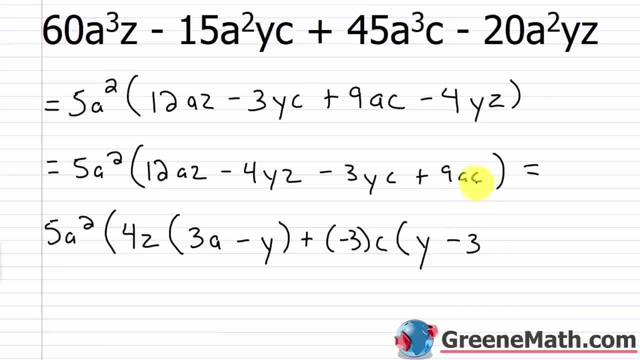 and then you'd have a 3 right. 9 over 3 is 3, and then the c would cancel. so you just have an a. now. I don't have a common binomial factor yet, but we're close. right, we have a y and a y. 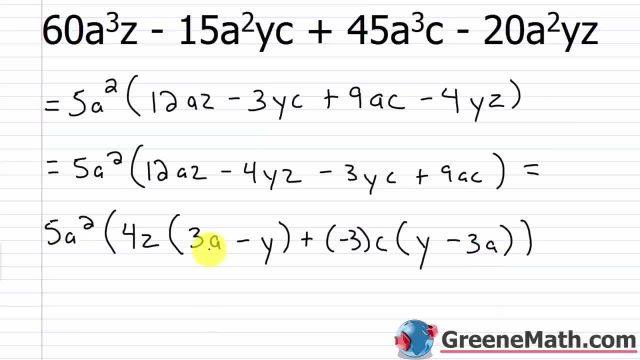 we have a 3a and a 3a. it's just the signs that are the problem. so if I was to factor out a negative here, if I was to factor out a negative here, then this sign would change and this sign would change. so, positive y and. 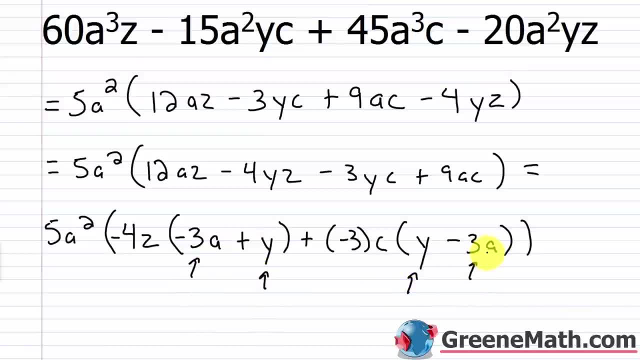 positive y, negative 3a and negative 3a. so that would work out. I just change the order. remember you can change the order, it won't matter. and let me just change the order here to y minus 3a. I know this is a little complex when you first see it, but 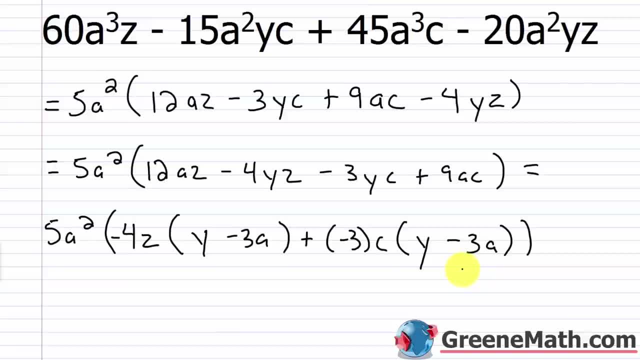 this is some of the problems that are going to get thrown at you right where you have to, you know, rework things and change the signs, and if you get something that's close, like we just got, it's usually just a sign that you're off by. so try a different sign. 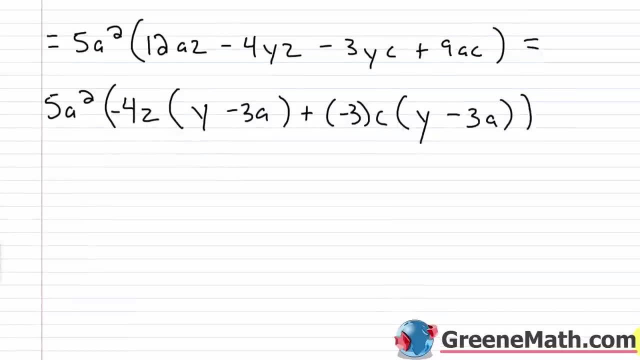 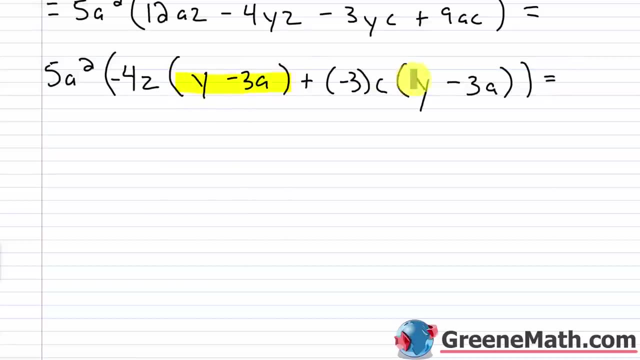 on each one. alright, so now we can go ahead and pull out our common binomial factor, which is y minus 3a, so I'll have my 5a squared out in front, not going to touch that inside. I'm pulling out the y minus 3a, so y minus. 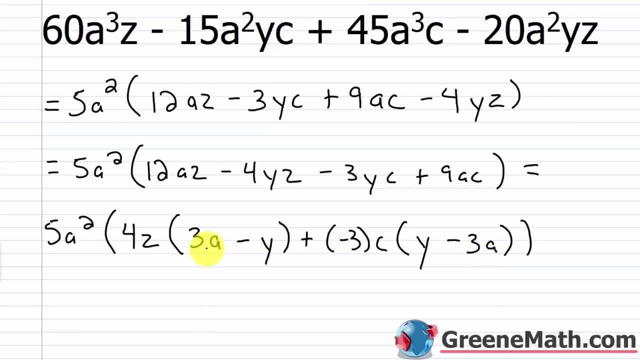 It's just the signs that are the problem. So if I was to factor out a negative here, if I was to factor out a negative here, then this sign would change, and this sign would change. So positive y and positive y, negative 3a and negative 3a. So that would work out. I just changed the order. Remember, you can change the order. It won't matter. 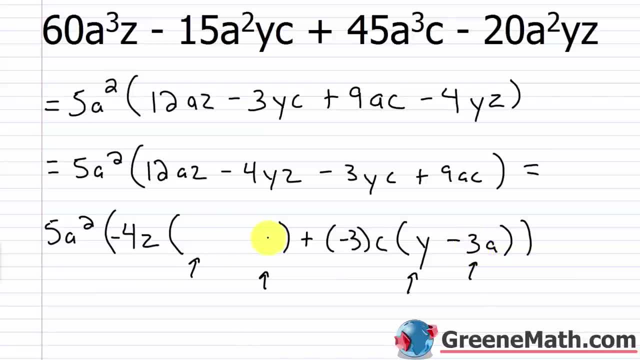 And let me just change the order here to y minus 3a. 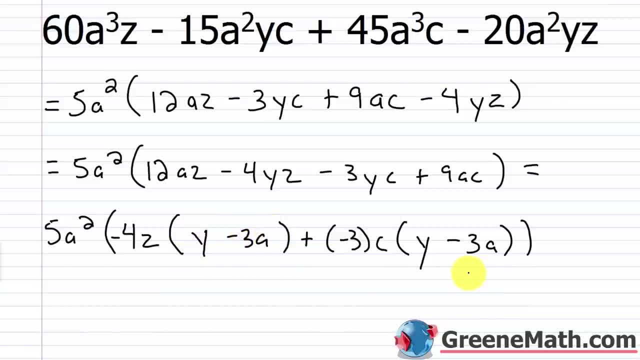 I know this is a little complex when you first see it, but this is some of the problems that are going to get thrown at you, right? 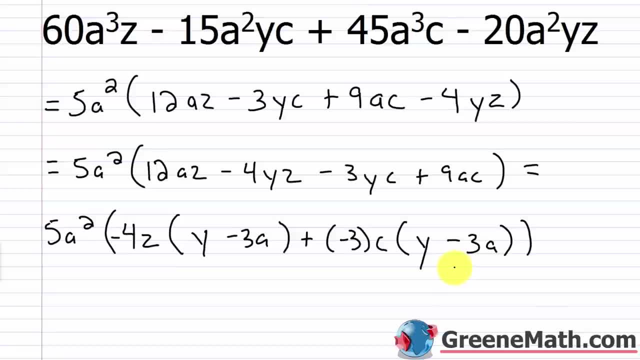 Where you have to, you know, rework things and change the signs. 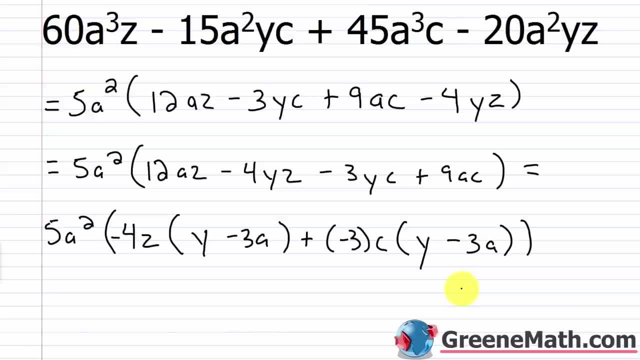 And if you get something that's close, like we just got, it's usually just a sign that you're off by. So try a different sign on each one. All right. 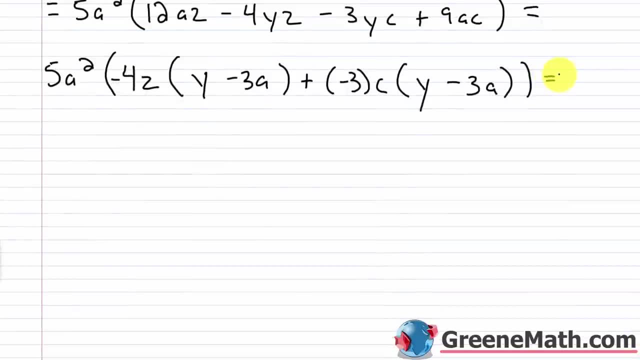 So now we can go ahead and pull out our common binomial factor, which is y minus 3a. So I'll have my 5a squared out in front. 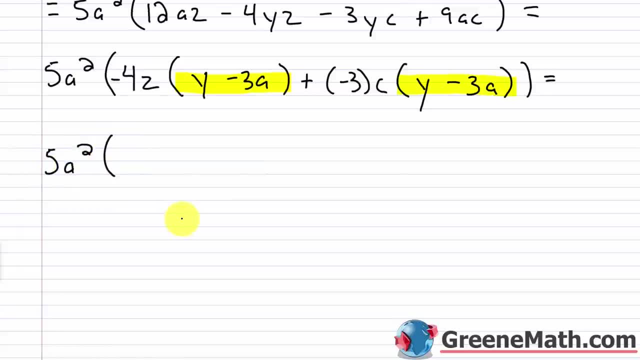 I'm not going to touch that. Inside, I'm pulling out the y minus 3a. So y minus 3a. And then what's left? If I pulled this out from here, 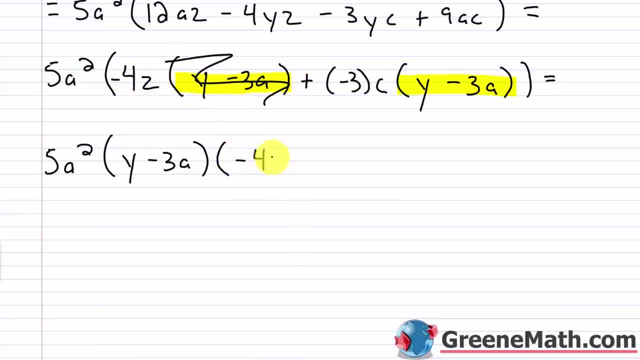 if I canceled it basically, I would have a negative 4z. And then I would have a minus 3c. This would be canceled if this was canceled. 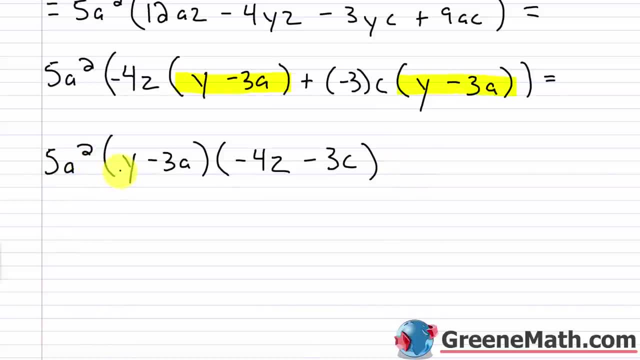 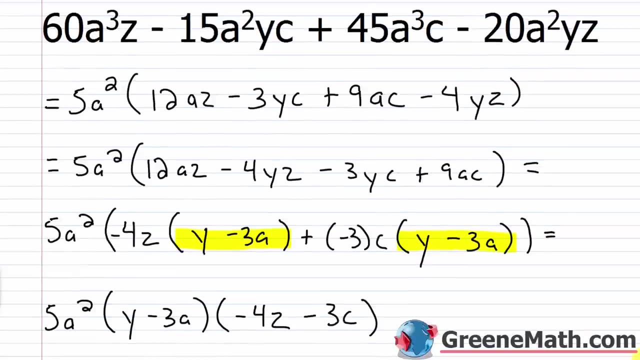 So I have my answer. 5a squared times the quantity y minus 3a times the quantity negative 4z minus 3c. And again, if you want to use FOIL here for these two and then multiply that result by 5a squared, you're going to see that you get this original four-term polynomial, 60a cubed z minus 15a squared yc, plus 45a cubed c minus 20a squared yz. 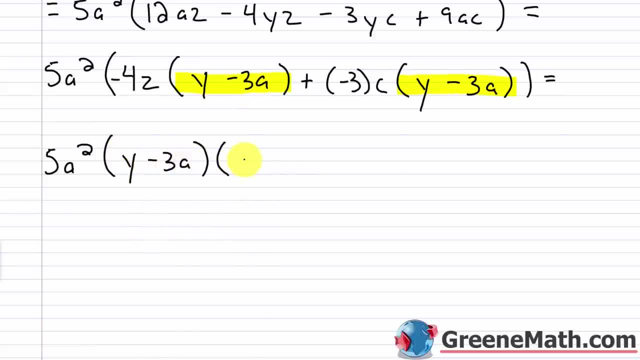 3a. and then what's left if I pulled this out from here, if I cancelled it, basically I would have a negative 4z and then I would have a minus 3c. this would be cancelled if this was cancelled. so I have my answer. 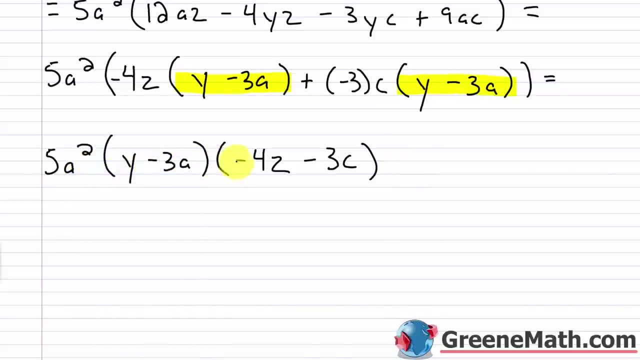 5a squared, times the quantity y minus 3a, times the quantity negative 4z minus 3c. and again, if you want to use foil here for these two and then multiply that result by 5a squared, you're going to see that you get this original. 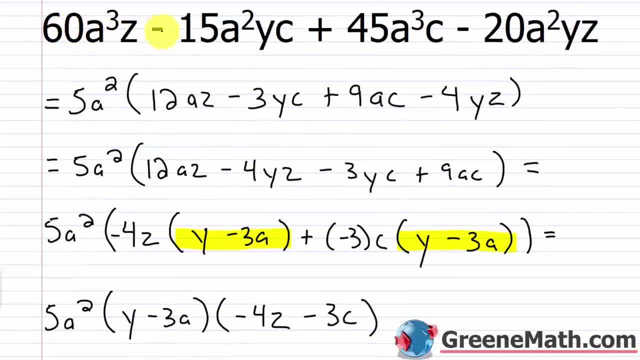 four term polynomial: 60a cubed z minus 15a squared yc, plus 45a cubed c minus 20a squared yz. and then one additional thing you might want to do, and I'm not sure if your teacher requires you to do this or not: 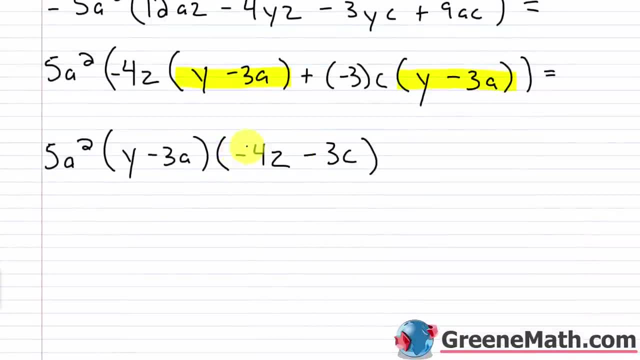 but a lot of times they don't like any of the leading terms in here to be negative. so you could further factor this and factor out a negative 1. so you could pull this guy out and this guy out and just change the sign. so I would just put a negative 1 all the way out. 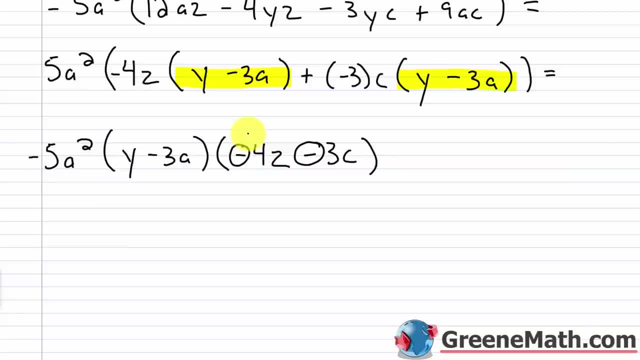 in front. so I just put a negative sign out here, and so this would turn into a positive, and then this would turn into a positive, and so you could also write the answer as negative. 5a squared times the quantity y minus 3a times the quantity. 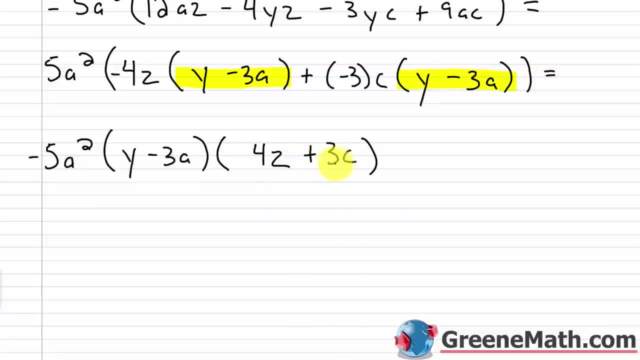 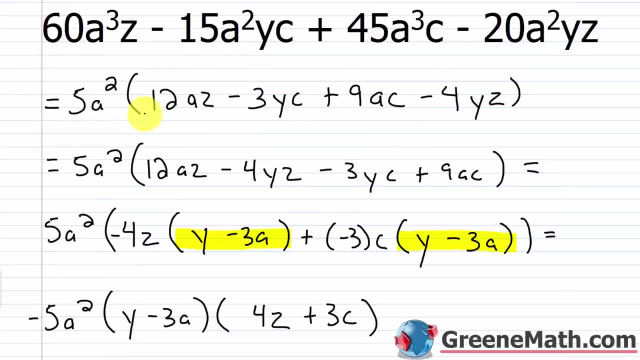 4z plus 3c. and again, if you go through and you multiply negative 5a, squared, times the quantity y minus 3a, and then you could do FOIL with that result. times this, you're going to get your original four term polynomial. 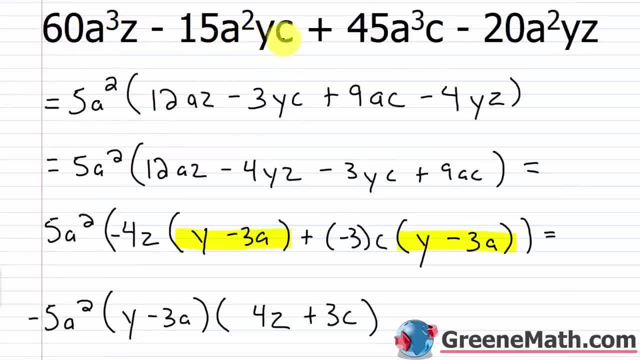 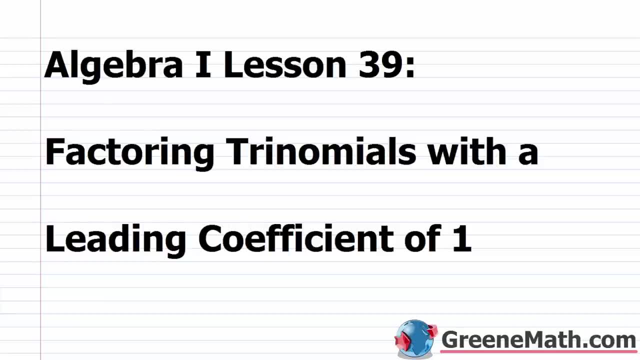 back the 60a cubed z minus 15a squared yc plus 45a cubed c minus 20a squared yc. hello and welcome to algebra 1, lesson 39. in this video we're going to learn about factoring trinomials with a leading coefficient. 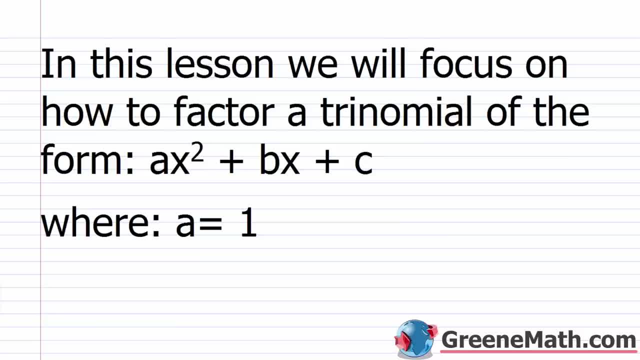 of 1. so before we kind of get started, I want you to recall that a trinomial is a polynomial with 3 terms. so in this lesson we will focus on how to factor a trinomial of the form we have ax squared plus bx. 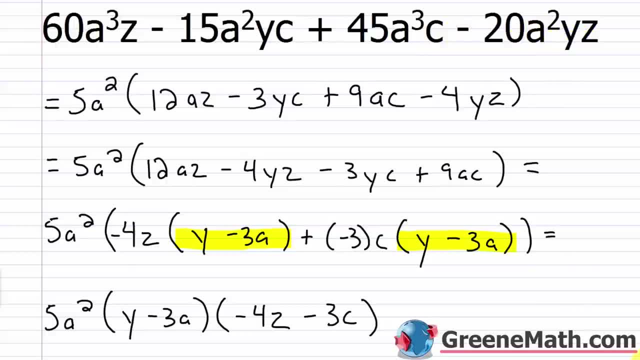 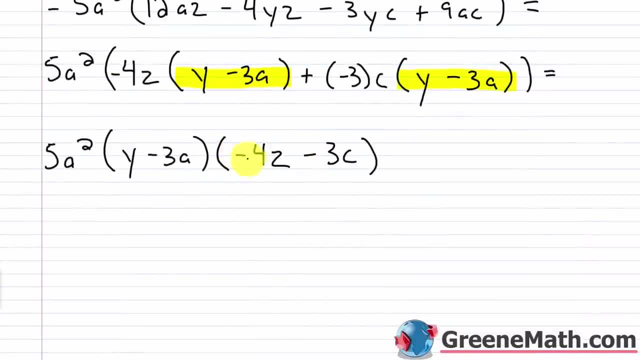 And then one additional thing you might want to do, and I'm not sure if your teacher requires you to do this or not, but a lot of times, they don't like any of the leading terms in here to be negative. So you could further factor this and factor out a negative 1. So you could pull this guy out and this guy out and just change the sign. So I would just put a negative 1 all the way out in front. So I just put a negative sign out here. 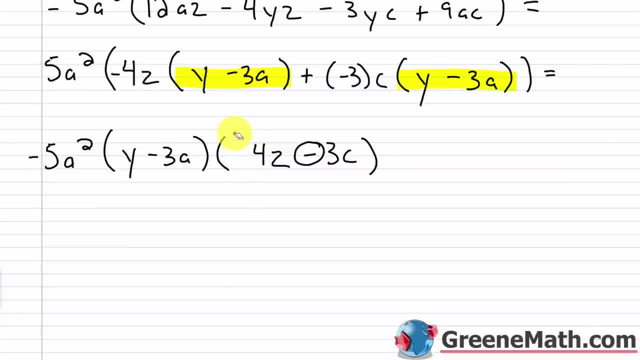 And so this would turn into a positive, and then this would turn into a positive. And so you could also write the answer 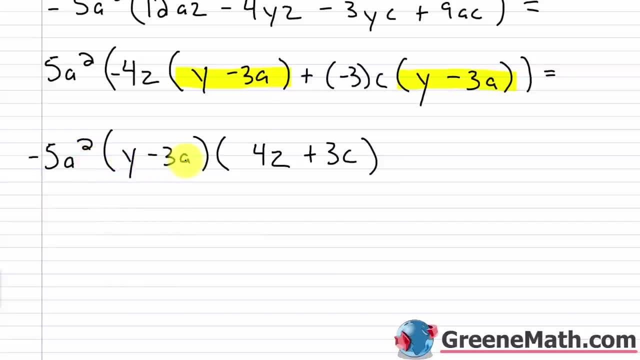 as negative 5a squared times the quantity y minus 3a times the quantity 4z plus 3c. 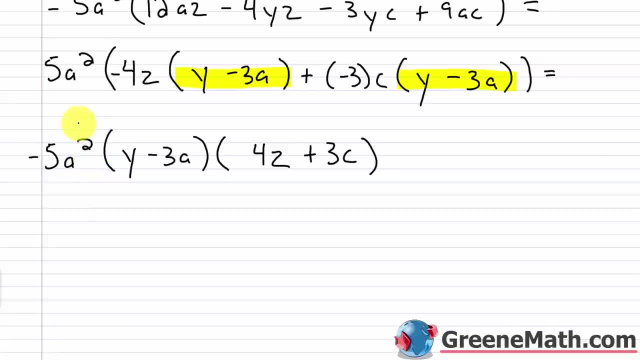 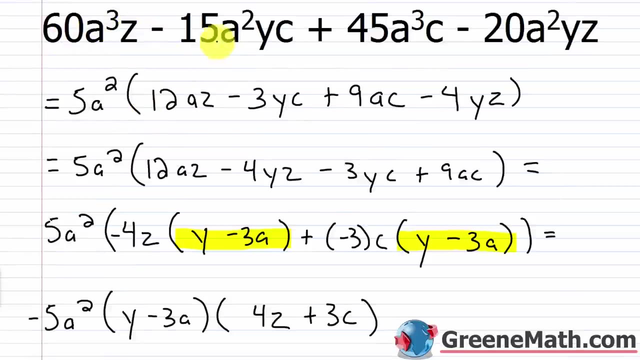 And again, if you go through and you multiply negative 5a squared times the quantity y minus 3a, and then you could do FOIL with that result times this, you're going to get your original four-term polynomial back, the 60a cubed z minus 15a squared yc plus 45a cubed c minus 20a squared yc. Hello, and welcome to Algebra 1, Lesson 39. 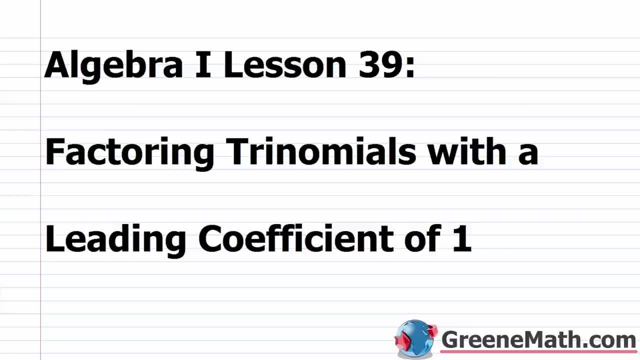 In this video, we're going to learn about factoring trinomials with a leading coefficient of 1. 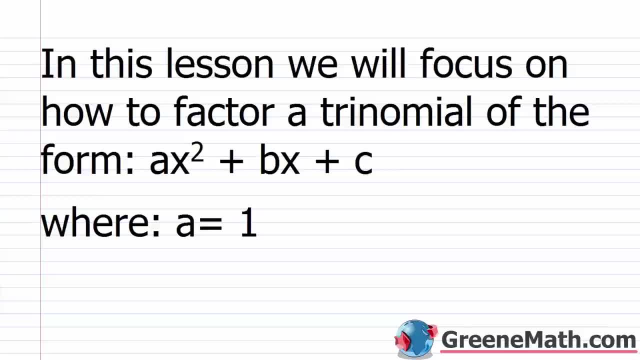 So before we kind of get started, I want you to recall that a trinomial is a polynomial with three terms. 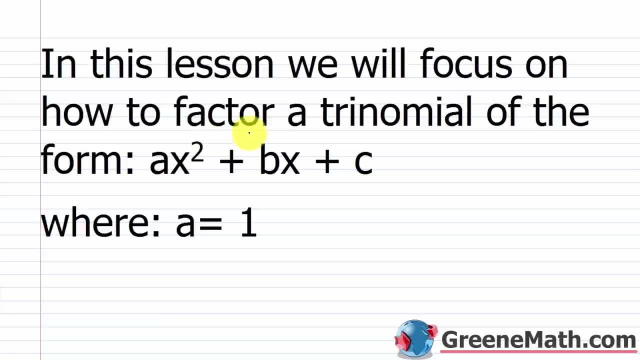 So in this lesson, we will focus on how to factor 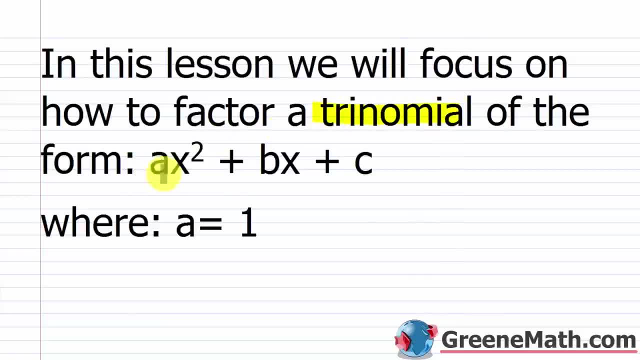 a trinomial of the form, we have ax squared plus bx plus c. 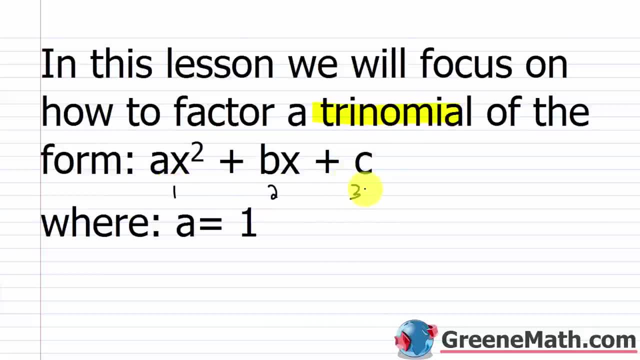 So again, you have one, two, three terms. Now, this is going to be the scenario that we're going to deal with today where a is always going to equal 1. So observe that a is the coefficient on the x squared term. b is the coefficient on the x term, right, the x to the first power term, and c is just a constant. 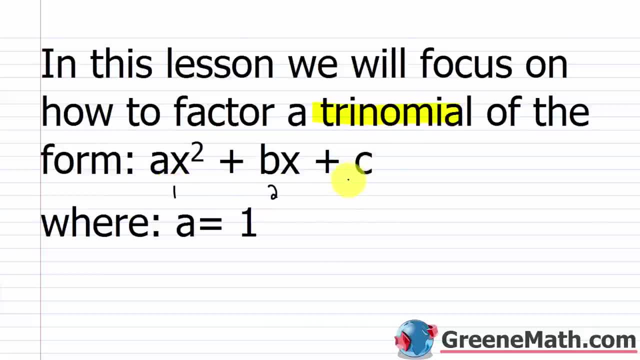 plus c. so again you have 1, 2, 3 terms. now this is going to be the scenario that we're going to deal with today, where a is always going to equal 1. so observe that a is the coefficient on the x squared term, b is the coefficient on 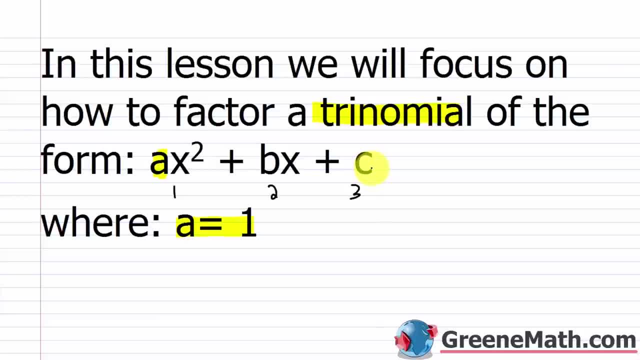 the x term, right the x to the first power term, and c is just a constant. so that's something I want you to memorize. I want you to write it down on a sheet of paper. I want you to look it over, because we're going to refer. 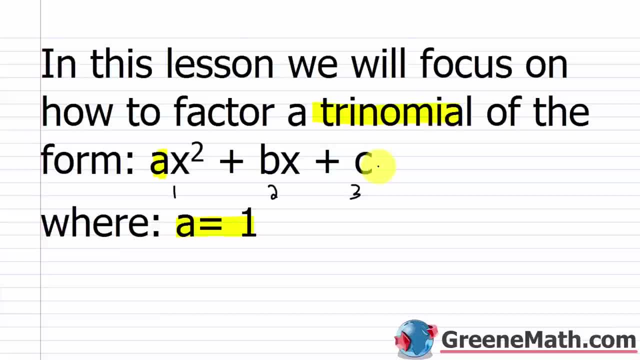 to that throughout this lesson and I don't want you to be lost. I'm going to talk about b and I'm going to talk about c, and so again, b is the coefficient for the x to the first power term and c is just the constant at the end of the trinomial. 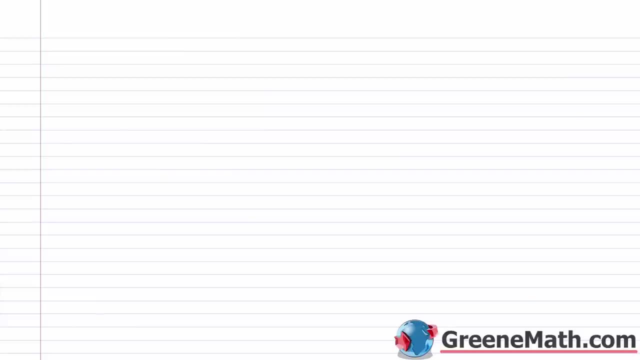 so we've already learned the basics of factoring and we're going to kind of take it one step further. so far we kind of know, you know, if I see something like 3x cubed minus 7x, that I can pull out an x that's common to both, so I can pull. 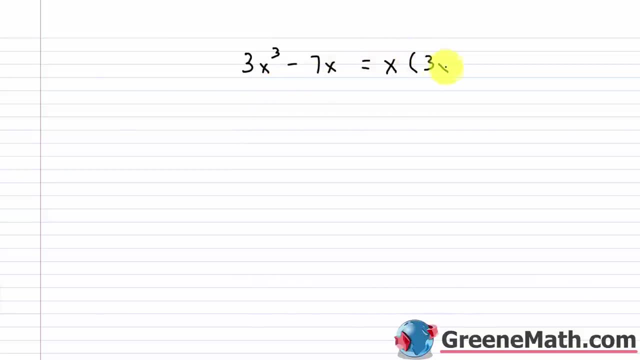 it out and write it outside of parentheses, and I would have 3x squared minus 7. alright, we know how to do that at this point. we also know how to do that if we have a common binomial factor. we learned that with factoring by grouping, but this is. 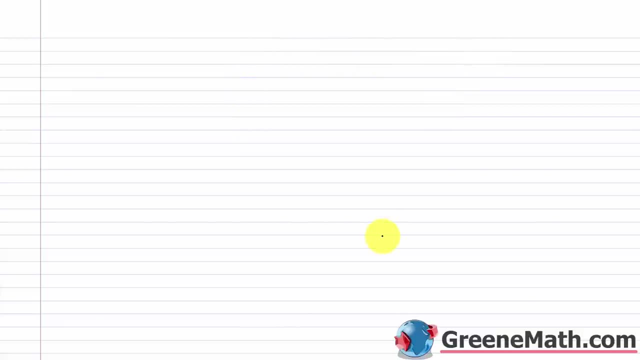 going to be something that's a little bit different. we're going to take a trinomial and we're going to factor it into the product of two binomials. right, remember, a binomial is a polynomial with two terms, so, in other words, we're. 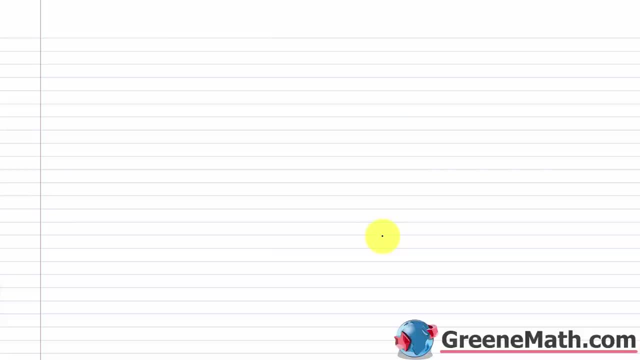 going to be reversing the FOIL process that we learned. so, for example, if I have something like x plus 3 times x plus 5, using FOIL we know that we can do the first terms: x times x is x squared. we can do the outer terms: x times 5 is plus 5x. 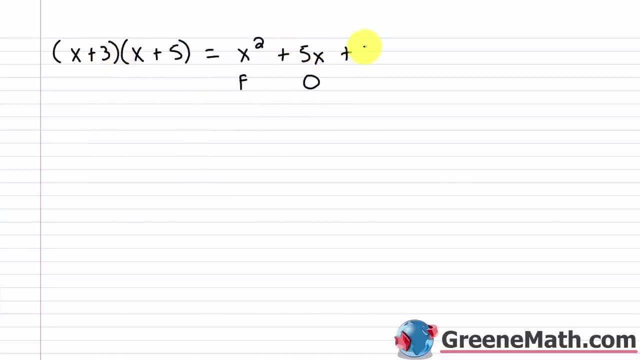 we can do the inside terms: 3 times x is plus 3x. and then we can do the last terms: 3 times 5 is plus 15. now, when we combine like terms here in the middle, we would end up with x squared plus 8x. 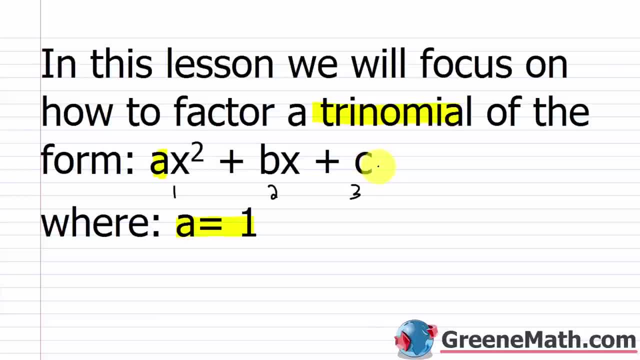 So that's something I want you to memorize. I want you to write it down on a sheet of paper. I want you to look it over because we're going to refer to that throughout this lesson, and I don't want you to be lost. 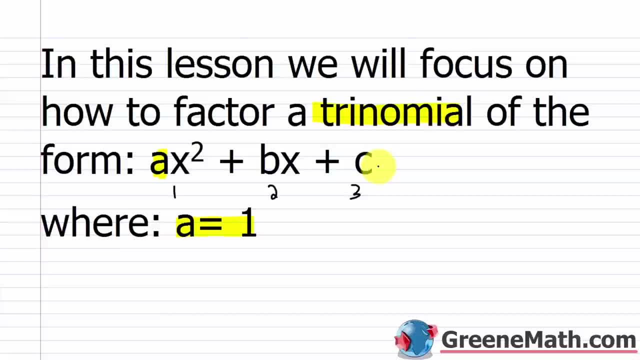 I'm going to talk about b, and I'm going to talk about c. And so again, b is the coefficient for the x to the first power term, and c is just the constant at the end of the trinomial. 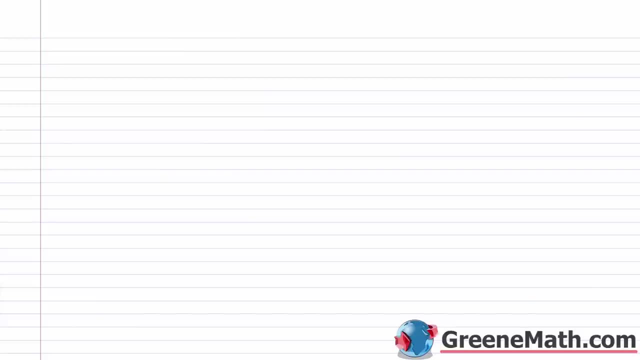 So we've already learned the basics of factoring, and we're going to kind of take it one step further. So far, we kind of know, you know, if I see something like 3x cubed, minus 7x, then I can pull out an x that's common to both. So I can pull it out and write it outside of parentheses, and I would have 3x squared minus 7. 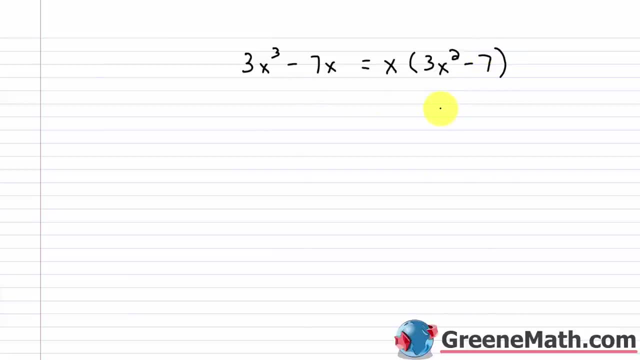 All right, we know how to do that at this point. We also know how to do that if we have a common binomial factor. 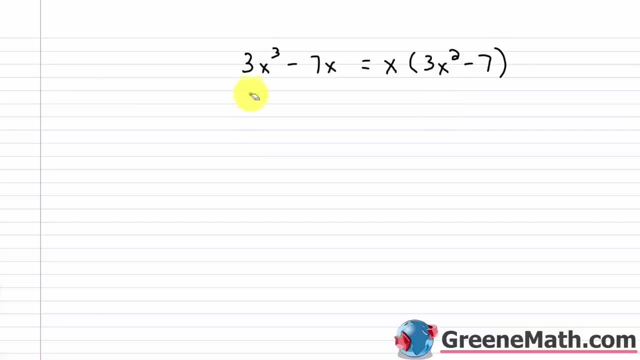 We learned that with factoring by grouping. But this is going to be something 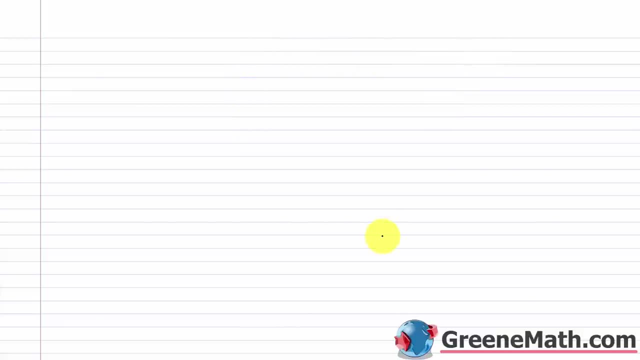 that's a little bit different. We're going to take a trinomial, and we're going to factor it into the product of two binomials, right? Remember, a binomial is a polynomial with two terms. 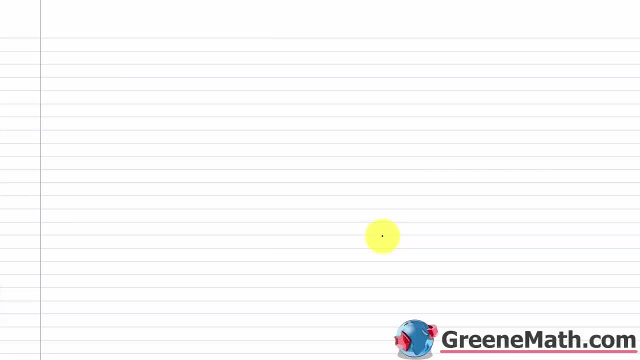 So in other words, we're going to be reversing the FOIL process that we learned. 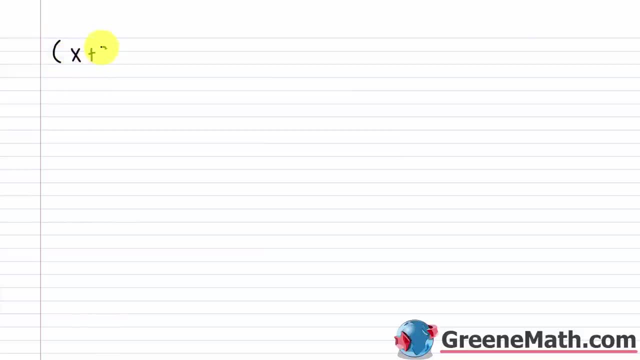 So for example, if I have something like x plus 3 times x plus 5, using FOIL, we know that we can do the first terms. x times x is x squared. We can do the outer terms. 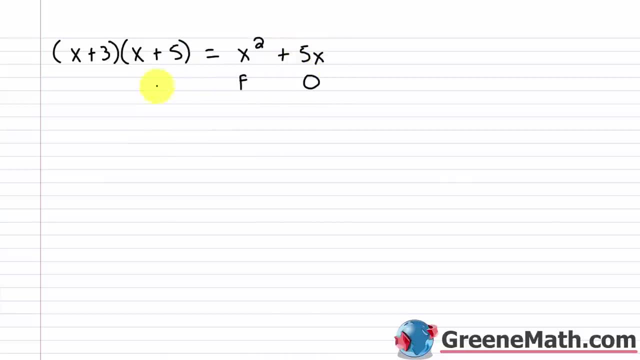 x times 5 is plus 5x. We can do the inside terms. 3 times x is plus 3x. 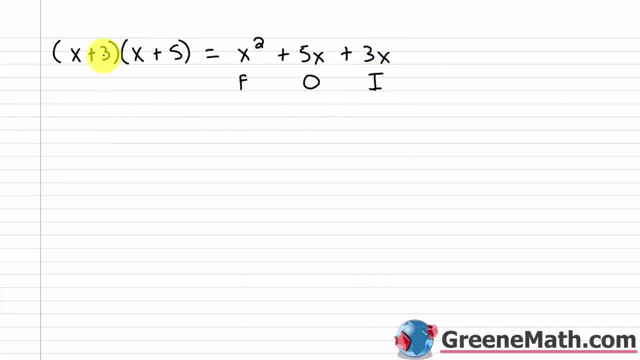 And then we can do the last terms. 3 times 5 is plus 15. 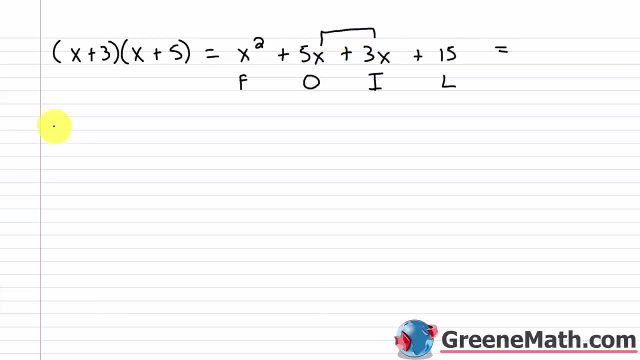 Now, when we combine like terms here in the middle, we would end up with x squared plus 8x plus 15. 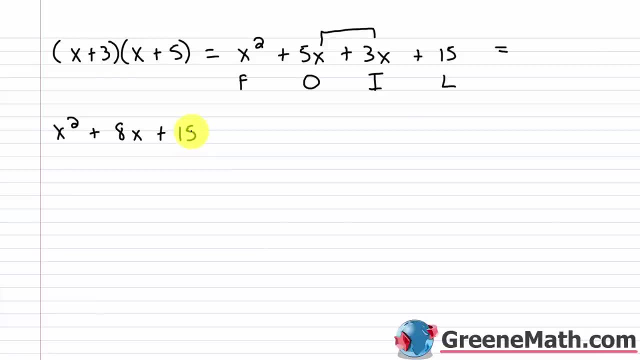 plus 15. now the question is, if I started out with this- this x squared plus 8x plus 15- and I asked you to go to this and you didn't have all this information, how would you go about doing it? well, the key here is to take this part. 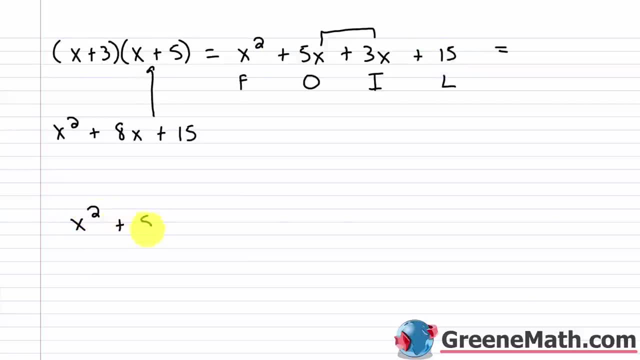 right here. so let's take the x squared plus 5x plus 3x plus 15 and let's write it in a different way. to make something obvious, we're going to factor out an x from these two middle terms, so x squared plus. I'm going to stick the x outside of a set of. 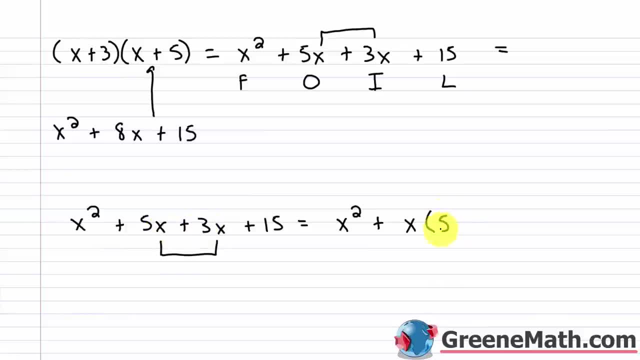 parentheses. it's common to both here. so 5 plus 3 and then plus 15. so the reason I'm doing that is to show you that these two integers here that we have inside the parentheses here, the 3 and the 5, these two guys are going to sum. 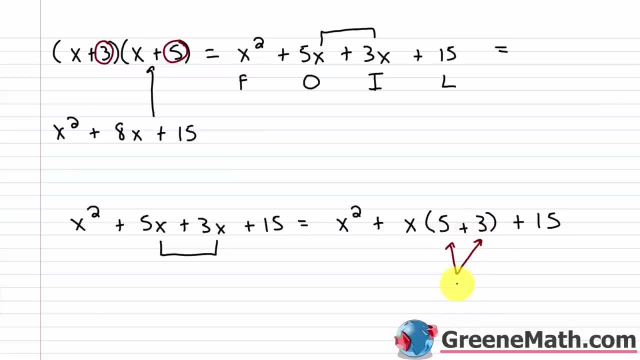 to give you your middle term in the trinomial. so these sum to give you 8. that's what we have here. so this, remember this- is the b. so we have ax squared plus bx plus c, so b, in this case, is going to be 8. so again, notice that those 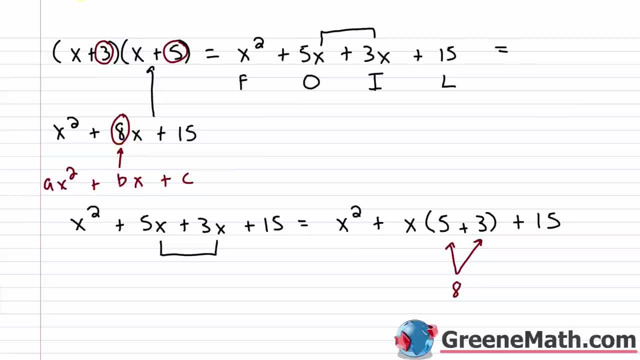 two integers sum to give you 8. now I want you to also notice that those same two integers multiply to give you 15. right c is 15 in this case. so two integers whose sum is b and whose product is c. that's what you're looking to find here. 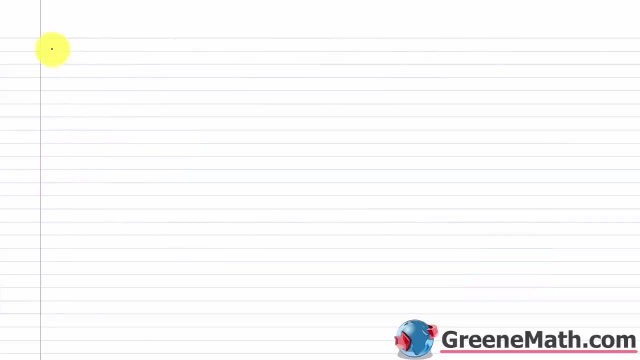 so let me erase this real quick. and let's say I started out with x squared plus 8x plus 15 and I said: go ahead and factor this into the product of two binomials. well, start with what you know. you know that you have two sets. 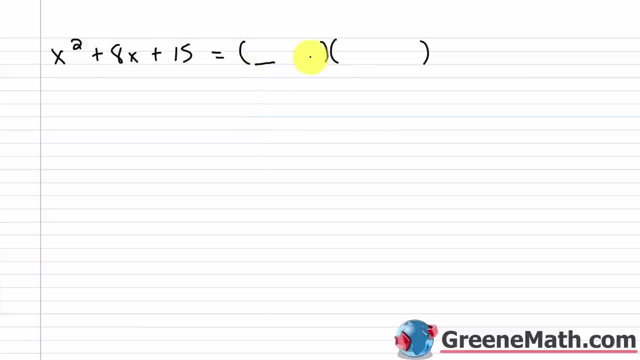 of parentheses like this and it's very, very easy to think about what goes here and here. remember: the first thing you do is you multiply the first terms together, the f in FOIL. so this times this would give you this. so x times x gives you x squared. 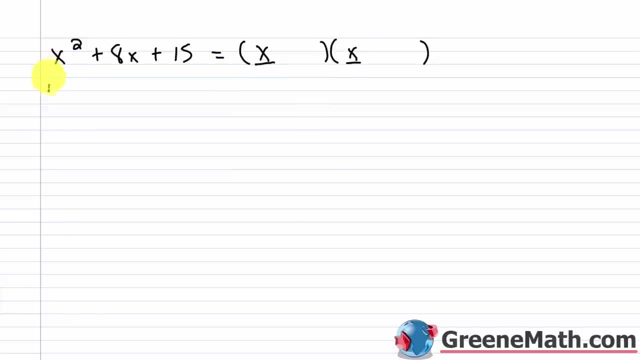 and that's always going to be the case. when your coefficient for the squared term is a 1 right, the first two positions are going to be that variable that you're working with raised to the first power. so, in other words, if this was p squared plus 8p, 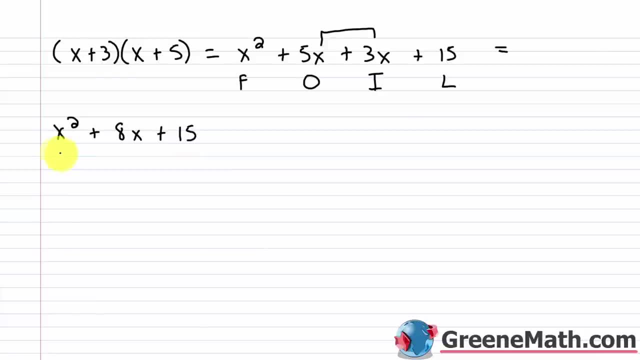 Now, the question is, if I started out with this, this x squared plus 8x plus 15, and I asked you to go to this, and you didn't have all this information, how would you go about doing it? 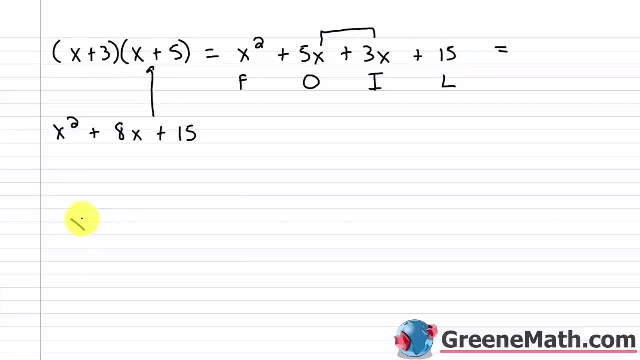 Well, the key here is to take this part right here. So let's take the x squared 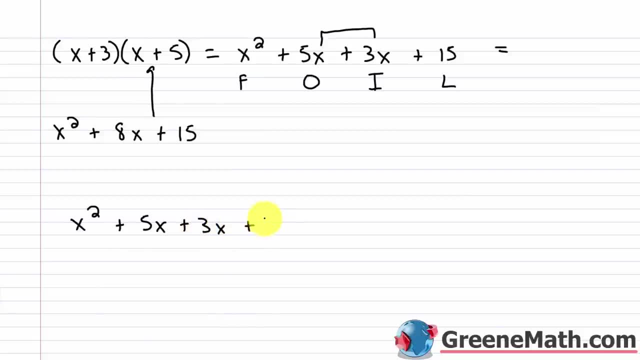 plus 5x plus 3x plus 15. 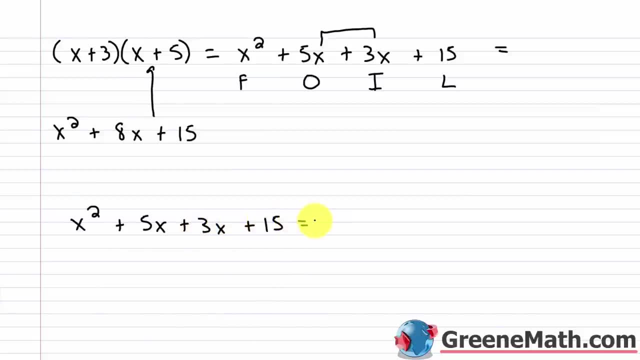 And let's write it in a different way to make something obvious. We're going to factor out an x from these two middle terms. So x squared plus, I'm going to stick the x outside of a set of parentheses. It's common to both here. So 5 plus 3 and then plus 15. 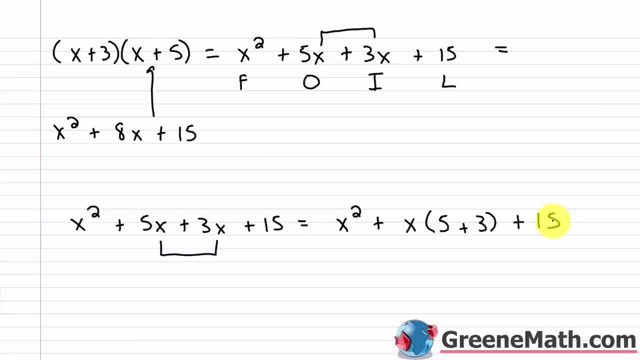 So the reason I'm doing that is to show you that these two integers here that we have inside the parentheses here, the 3 and the 5, these two guys are going to sum to give you your middle term in the trinomial. So these sum to give you 8. That's what we have here. 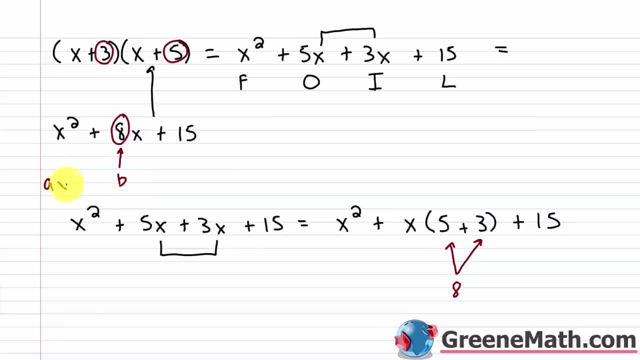 So this, remember, this is the b. So we have ax squared plus bx plus c. So b in this case is going to be 8. 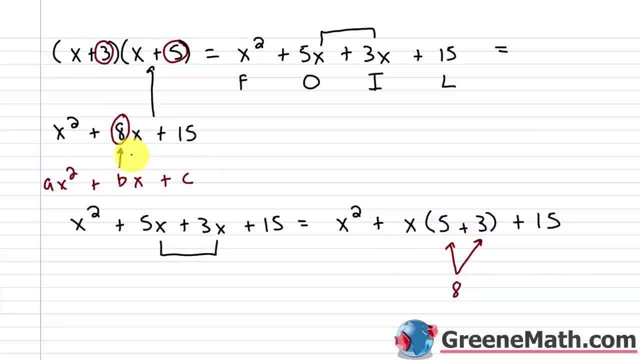 So again, notice that those two integers sum to give you 8. 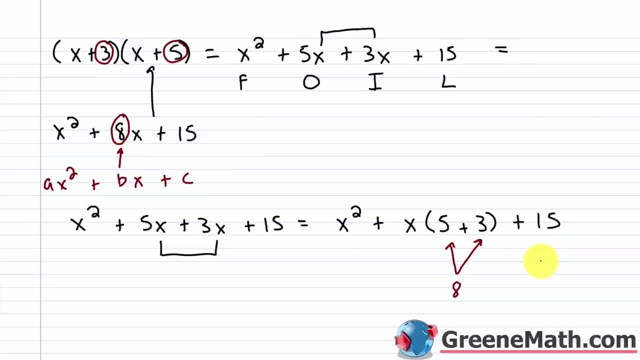 Now I want you to also notice that those same two integers multiply to give you 15. 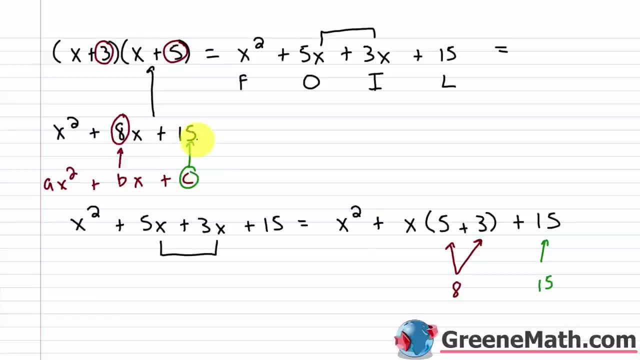 Right, c is 15 in this case. So two integers whose sum is b and whose product is c. That's what you're looking to find here. 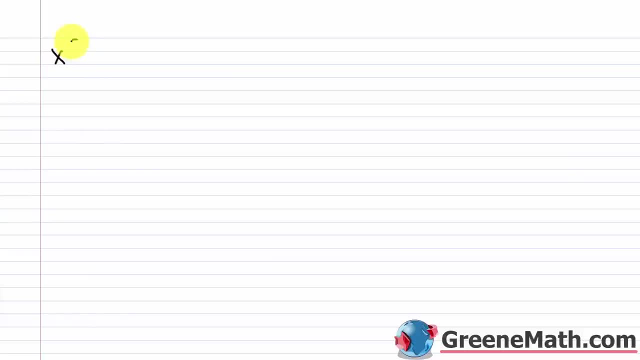 So let me erase this real quick. And let's say I started out with x squared plus 8x plus 15. And I said, go ahead and factor this into the product of two binomials. 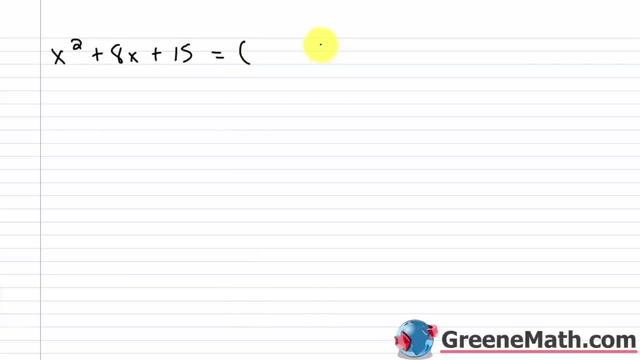 Well, start with what you know. You know that you have two sets of parentheses like this. And it's very, very easy to think about what goes here and here. 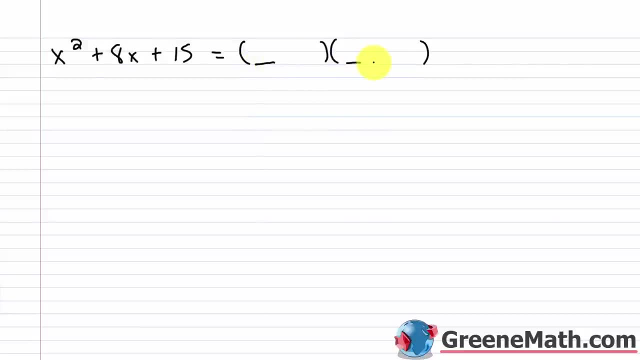 Remember, the first thing you do is you multiply the first terms together. The f in FOIL. So this times this would give you this. 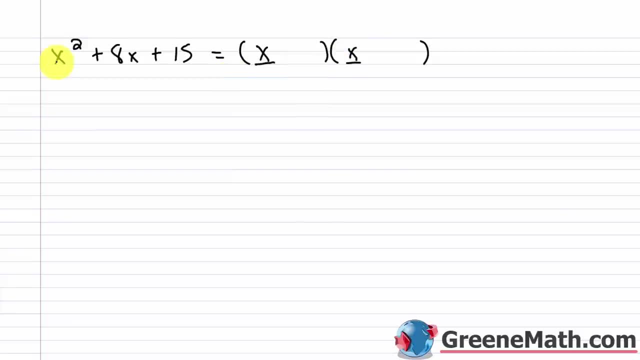 So x times x gives you x squared. And that's always going to be the case when your coefficient for this for the square term is a 1. Right, the first two positions are going to be that variable that you're working with raised to the first power. 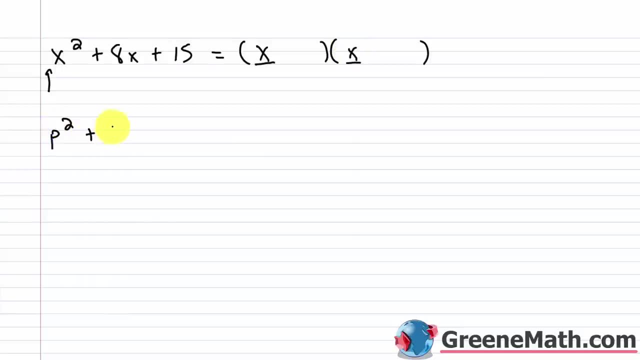 So in other words, if this was p squared plus 8p plus 15, well then the first two positions in this case would be p and p. Right, it's the same thing. Just changing the variable up. 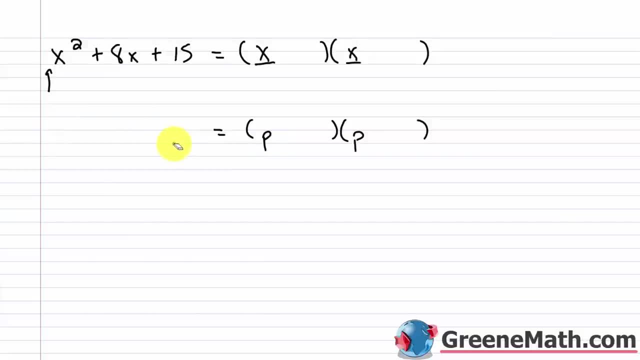 Do the same thing now. Or if I had something like 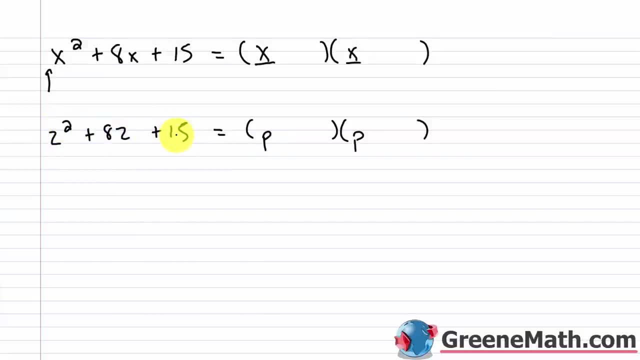 z squared plus 8z plus 15, then this would be z. And this would be z. 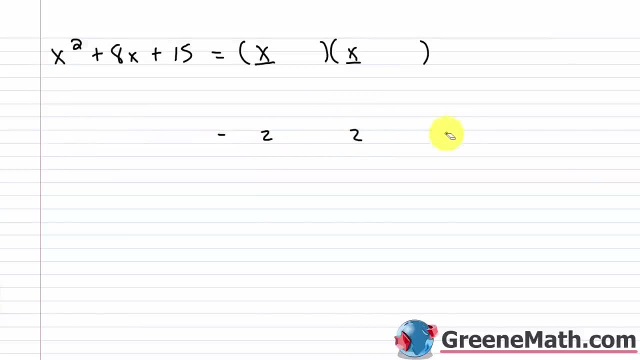 Right, very, very straight forward. Okay, so once we've figured that part out, that part's a given. 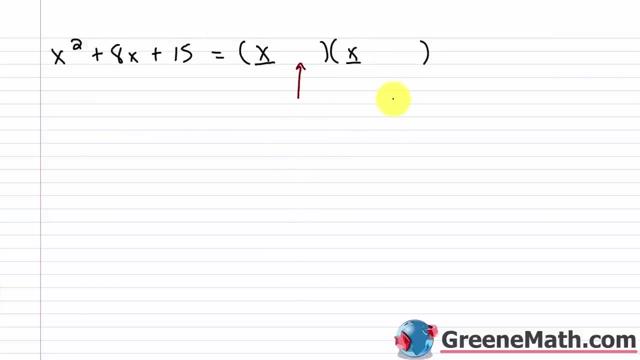 So the question is how do I find out what goes here and here? 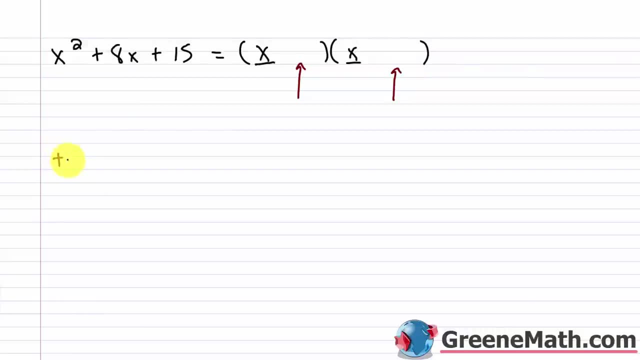 Well again, I want two integers. So let me write this out. Two integers where the sum is going to be b and the product is going to be c. 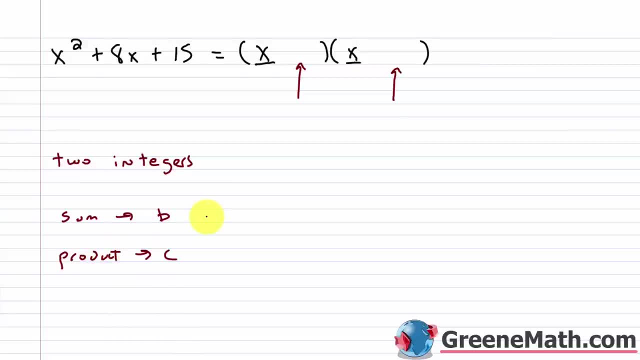 So we already know at this point that those two integers are 5 and 3. Right, they sum to b. Remember this is b. 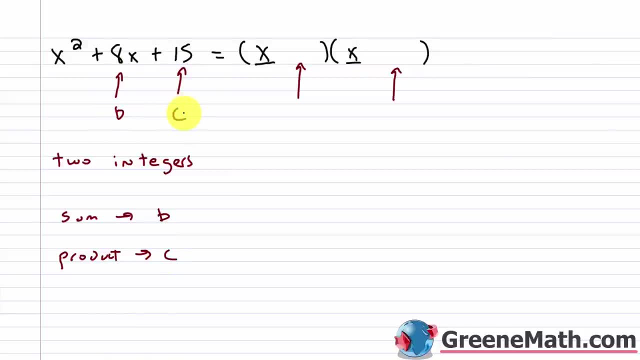 And the product is c. Remember this is c. So 5 times 3 is 15. Again, 5 plus 3 is 8. So those are the two numbers we're looking for. Once we find them, we can just write them in any order. 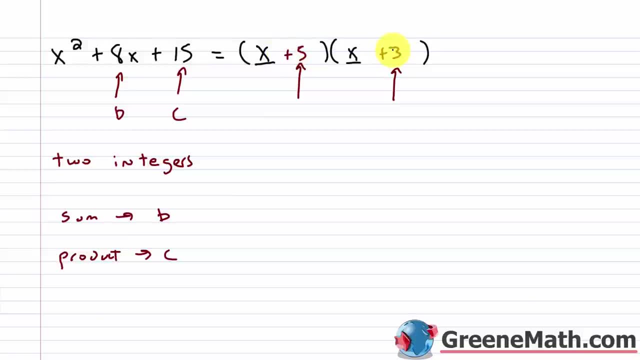 I could put plus 5 and plus 3. Or I could switch that up and put plus 3 and plus 5. 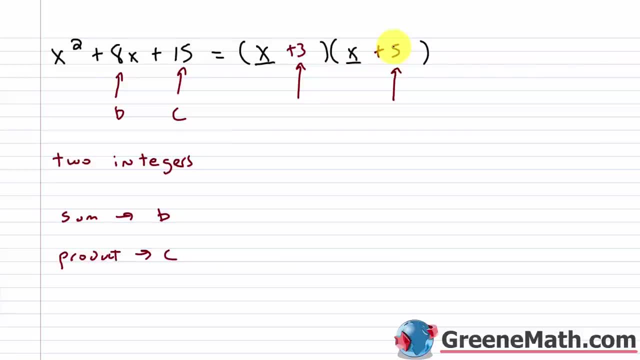 And you have successfully factored this. Right, we know through FOIL x times x is x squared. 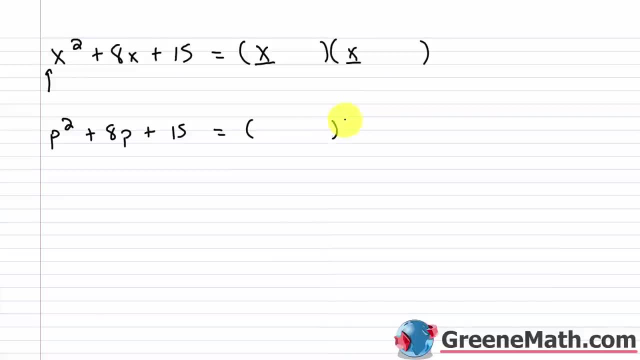 plus 15. well then, the first two positions in this case would be p and p. right, it's the same thing, just changing the variable up. do the same thing now. or if I had something like z squared plus 8z plus 15, then this would be z. 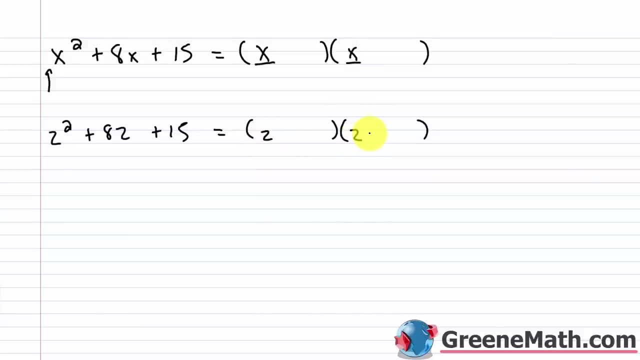 and this would be z right very, very straight forward. ok, so once we've figured that part out, that part's a given. so the question is: how do I find out what goes here and here? well, again, I want two integers. so let me write this out: two integers. 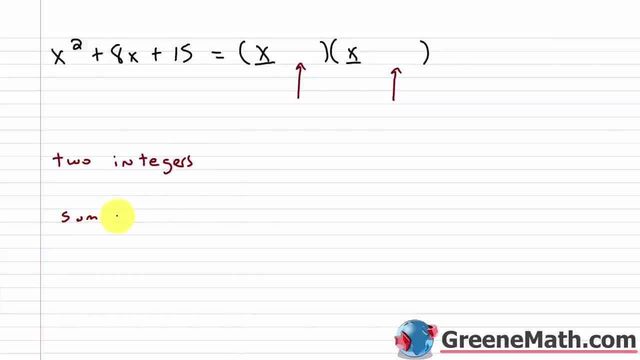 where the sum is going to be b and the product is going to be c. so we already know at this point that those two integers are 5 and 3. right, they sum to b- remember this is b- and the product is c- remember this is c. so 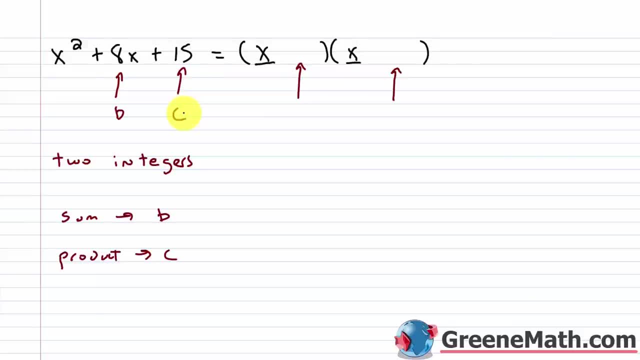 5 times 3 is 15. again, 5 plus 3 is 8. so those are the two numbers we're looking for. once we find them, we can just write them in any order. I could put plus 5 and plus 3, or I could switch that up and put: 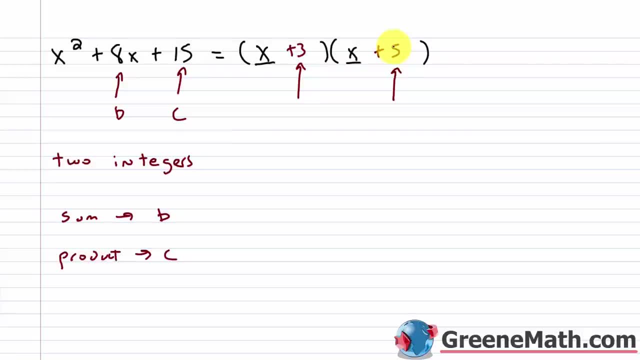 plus 3 and plus 5, and you have successfully factored this right. we know through FOIL, x times x is x. squared x times 5 is plus 5x. 3 times x is plus 3x. combine like terms there, you get plus 8x, and then we have: 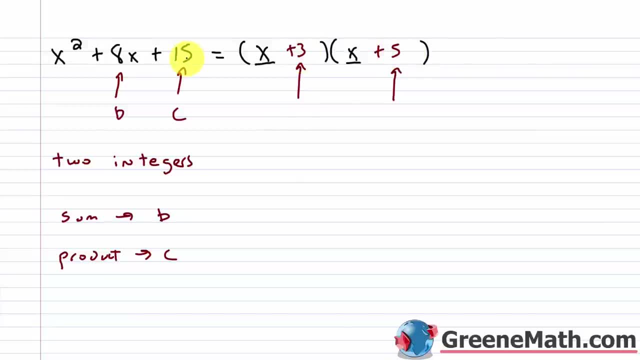 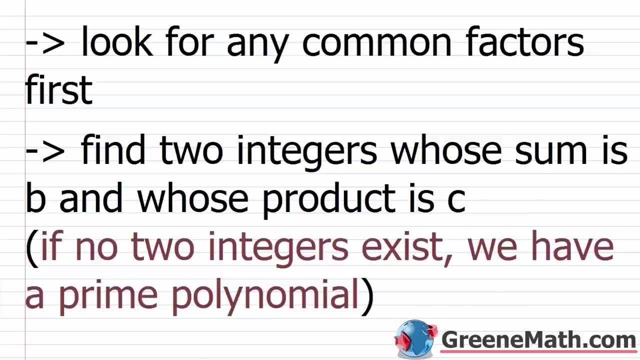 plus 3 times plus 5, that would be positive 15, and so you get this trinomial x squared plus 8x plus 15 back. so let's just quickly run down the official procedure. so for factoring a trinomial, again with a. 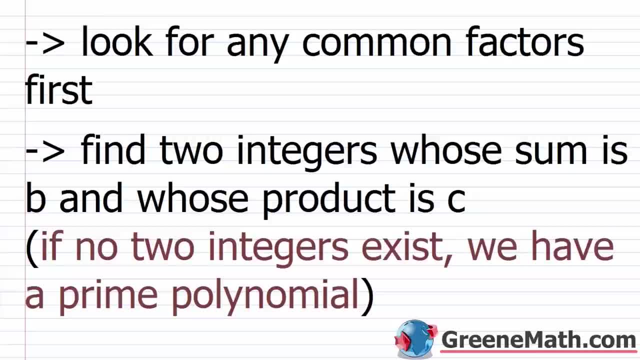 leading coefficient of 1, so that a is equal to 1. you're going to look for any common factors first. so just like we saw with factoring by grouping, you know if you had something like, let's say, 2x squared plus 6x plus 8. 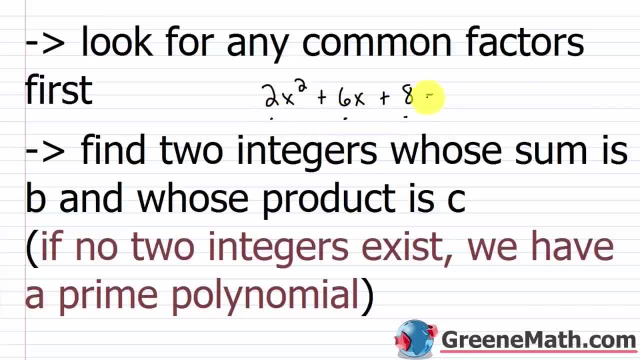 I have a common factor of 2 and I could start out by just pulling that outside the parentheses. so 2 times the quantity x squared plus 3x plus 4. I would start out by doing that and then I would factor what's inside the parentheses into the product. 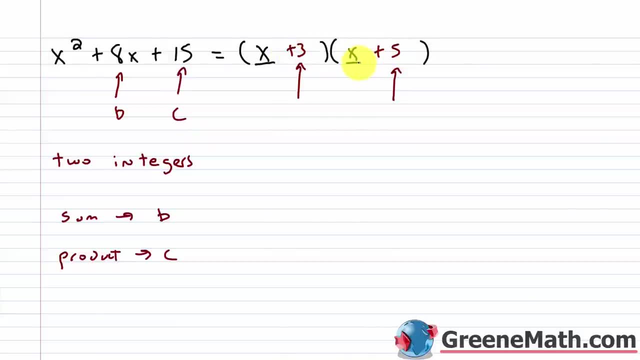 x times 5 is plus 5x. 3 times x is plus 3x. Combine like terms there, you get plus 8x. And then we have plus 3 times plus 5. That would be positive 15. And so you get this trinomial x squared plus 8x plus 15 back. So let's just quickly run down the official procedure. 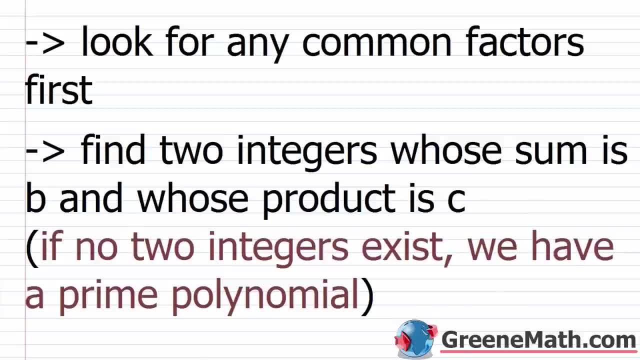 So for factoring a trinomial, again with a leading coefficient of 1, so that a is equal to 1, you're going to look for 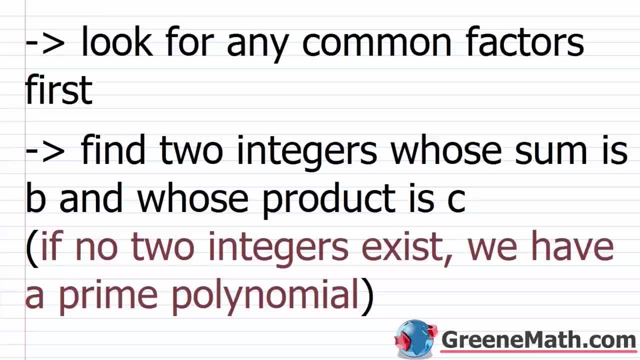 any common factors first. So just like we saw with factoring by grouping, if you had something like 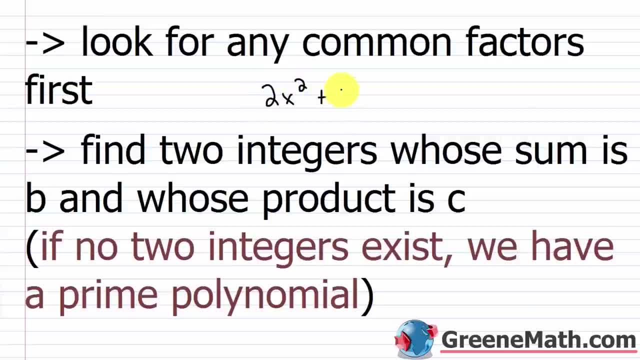 let's say 2x squared plus 6x plus 8, I have a common factor of 2. 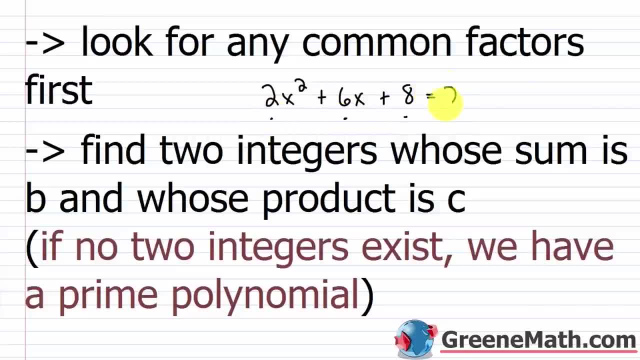 And I could start out by just pulling that outside the parentheses. 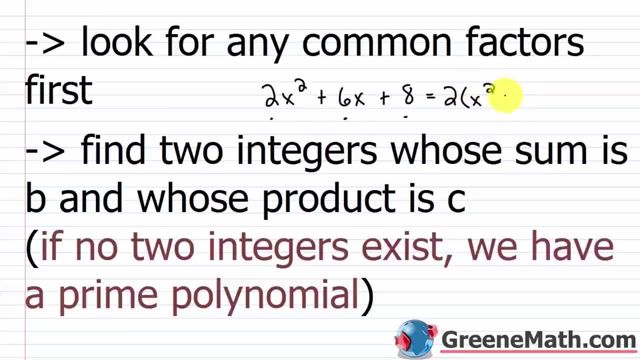 So 2 times the quantity x squared plus 3x plus 4. I would start out by doing that. And then I would factor 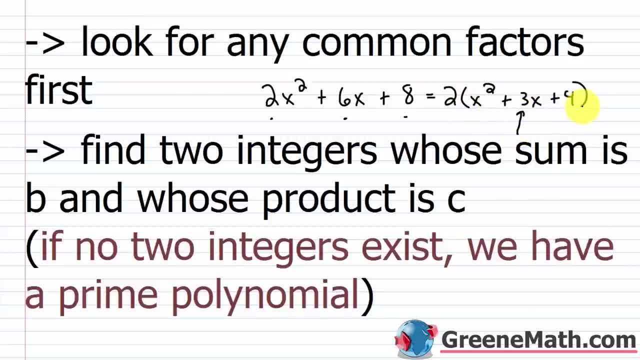 what's inside the parentheses into the product of two binomials. 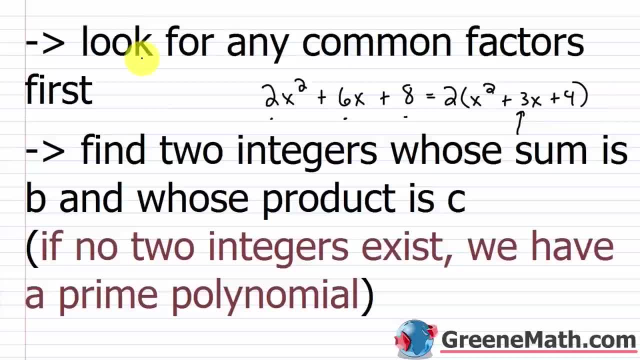 So once I've done this, once I've looked for any common factors and if they exist, pulled them out, I want to again find two integers whose sum is b. Remember that's the coefficient for the x to the first power term and whose product is c. Remember that's your constant at the end. 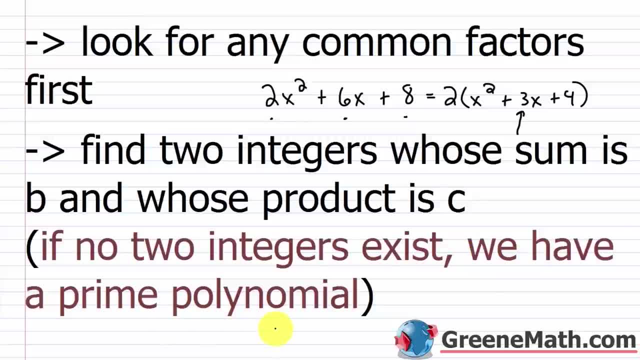 If no two integers exist, we have a prime polynomial. 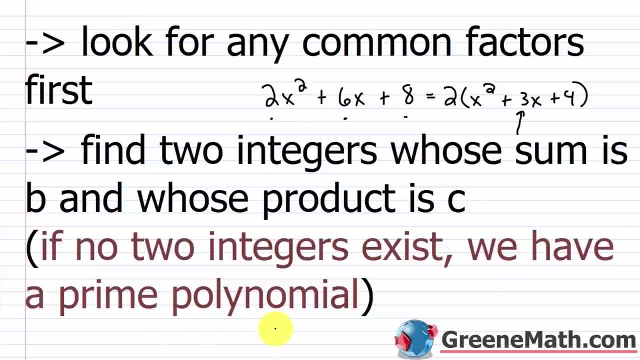 So at this point, we're not going to be able to factor that. Alright, let's take a look at the first one. So we have p squared plus 18p squared. Plus 80. 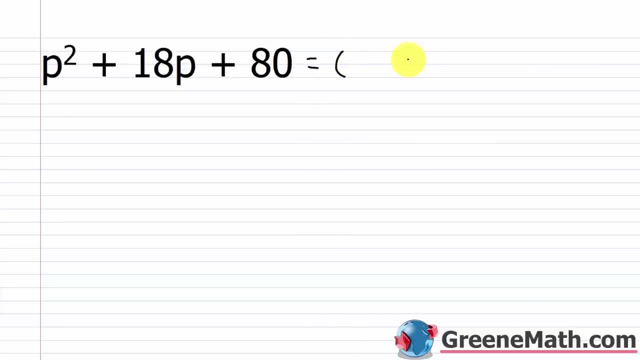 So again, when you first start out, just go ahead and put two sets of parentheses. I notice that there's nothing common to everything. So there's nothing to pull out to start. 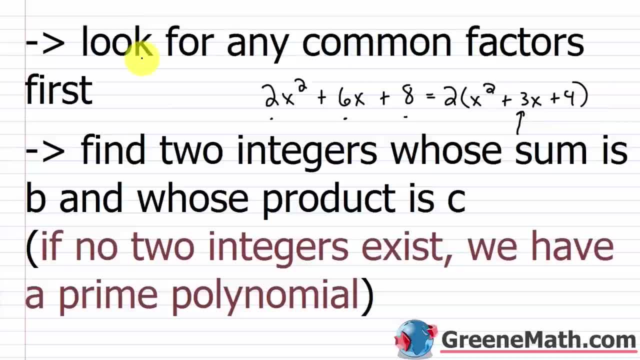 of two binomials. so once I've done this, once I've looked for any common factors and, if they exist, pulled them out, I want to again find two integers whose sum is b- remember that's the coefficient for the x- to the first power term- and whose product. 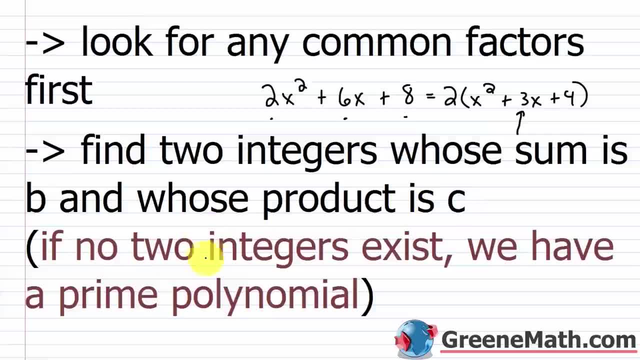 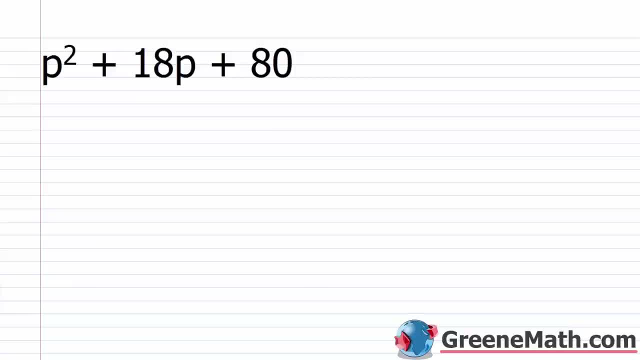 is c. remember, that's your constant. at the end, if no two integers exist, we have a prime polynomial. so at this point we're not going to be able to factor that. alright, let's take a look at the first one. so we have p squared plus 18p plus 80. 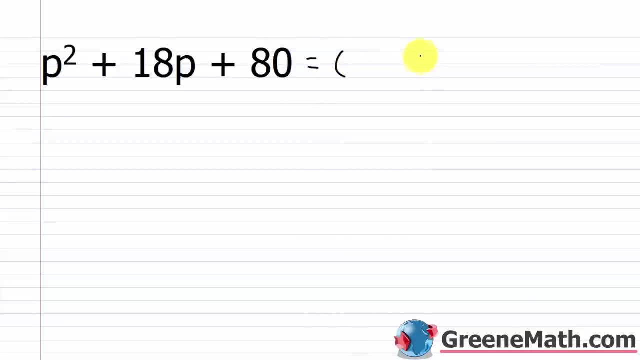 so, again, when you first start out, just go ahead and put two sets of parentheses. I notice that there's nothing common to everything, so there's nothing to pull out to start, and so I know that here and here is a given right. if this is a 1 right there, then it's just going to be. 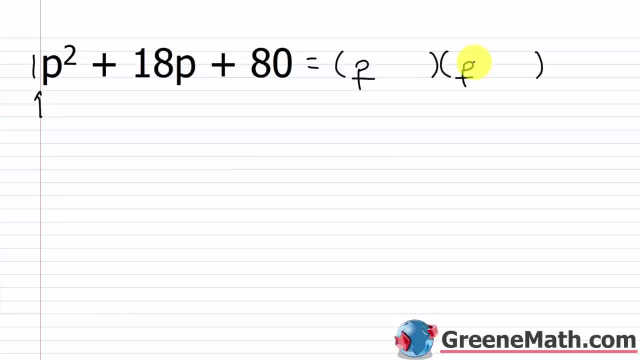 p times p. very, very easy to get the first ones. then after that, I'm again looking for these two positions right here. so give me two integers: whose sum is this and whose product is this? so what you need to do is start thinking about the factors of 80. 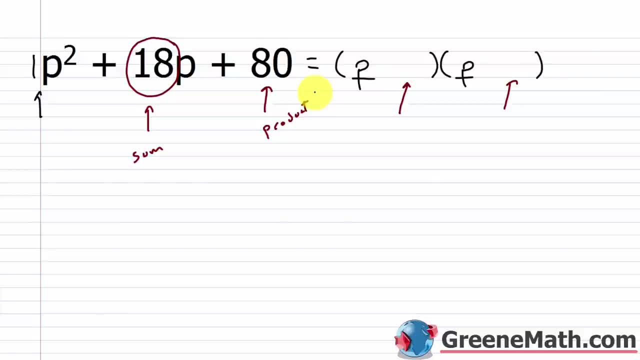 well, you could make a factor tree if you wanted to, and sometimes that's necessary- or you kind of just on your scratch paper, go okay. well, I got 1 and 80. that's obviously too far apart. to sum to 18, I've got 2. 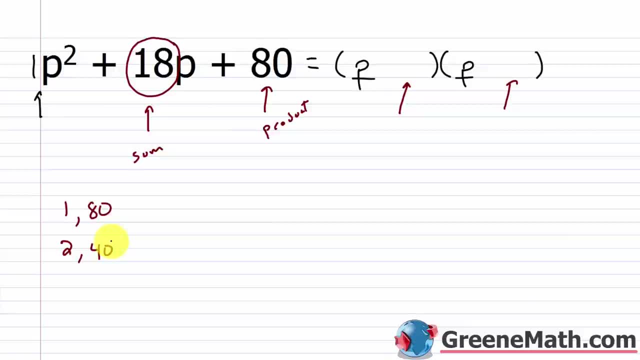 and 40. again that's too far apart. 80 is not divisible by 3. I've got 4 and 20- again too far apart. I've got 5 and 16. that's not going to work for a sum then. I've got not divisible by 6, not. 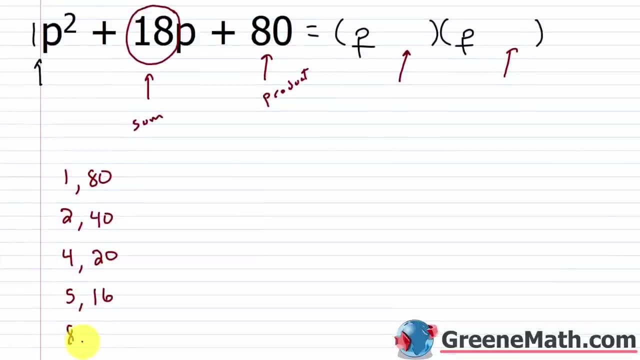 divisible by 7, but is divisible by 8, 8 and 10. so I've found two numbers whose product is 80, 8 times 10 is 80 and whose sum is 18. 8 plus 10 is 18. once you've found, 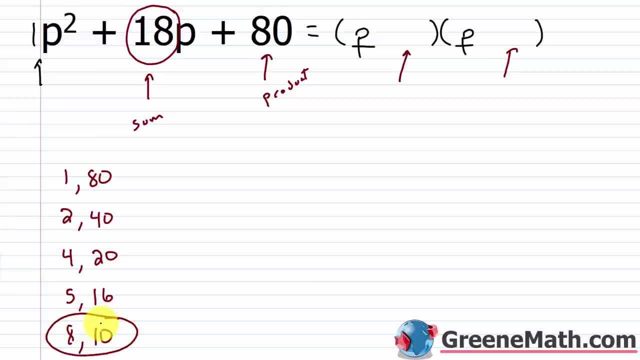 that you can go ahead and stop. so I have my combination here and again. I could write this in any order. I could put plus 8 here, plus 10 here, or I could reverse it and I could go. you know, plus 10, plus 8, doesn't matter. now I. 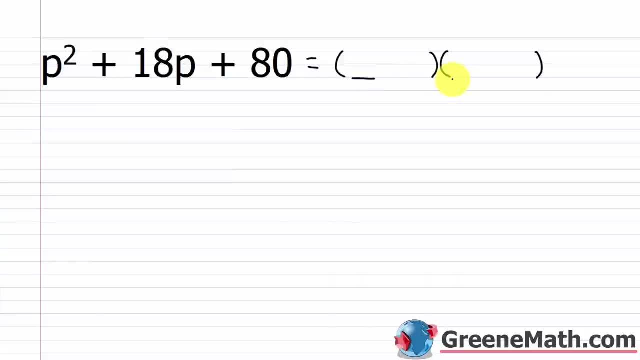 And so I know that here and here is a given, right? If this is a one right there, then it's just going to be p times p. Very, very easy to get the first ones. Then after that, I'm again looking for these two positions right here. 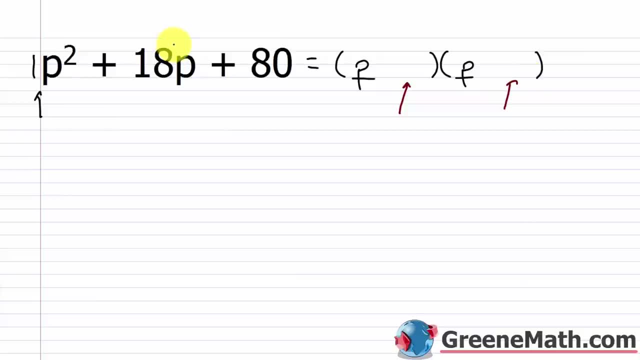 So give me two integers. Whose sum is this? 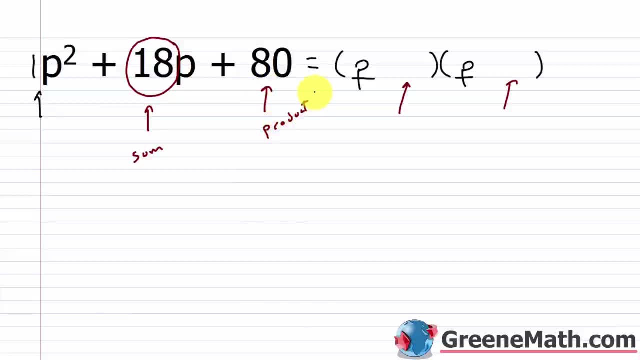 And whose product is this? So what you need to do is start thinking about the factors of 80. Well, you could make a factor tree if you wanted to, and sometimes that's necessary. Or you kind of just on your scratch paper go, OK, well, I got 1 and 80. That's obviously too far apart to sum to 18. I've got 2 and 40. Again, that's too far apart. 80 is not divisible by 3. I've got 4 and 20. Again, too far apart. 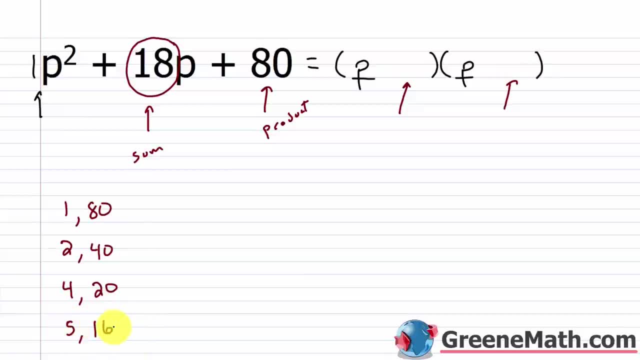 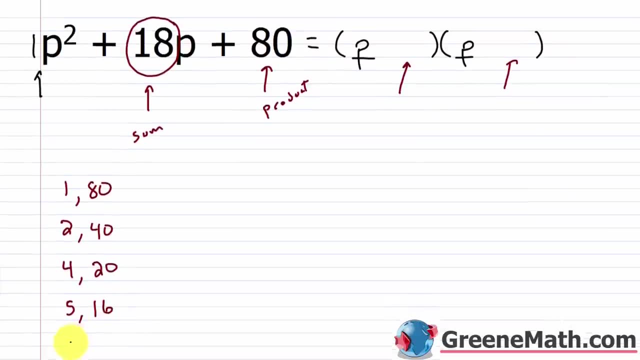 I've got 5 and 16. That's not going to work for a sum. Then I've got not divisible by 6, not divisible by 7, but is divisible by 8. 8 and 10. So I've found two numbers whose product is 80. 8 times 10 is 80. And whose sum is 18. 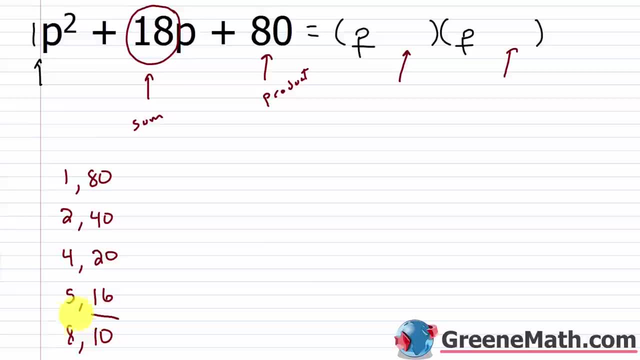 Once you've found that, you can go ahead and stop. So I have, my combination here. And again, I could write this in any order. 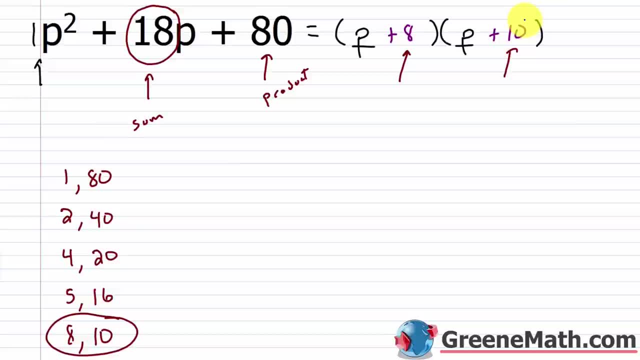 I could put plus 8 here, plus 10 here, or I could reverse it and I could go, you know, plus 10, plus 8. Doesn't matter. Now, I like to check things. Those of you who watch my videos know that. So let's spend a little bit of time here and just check it. 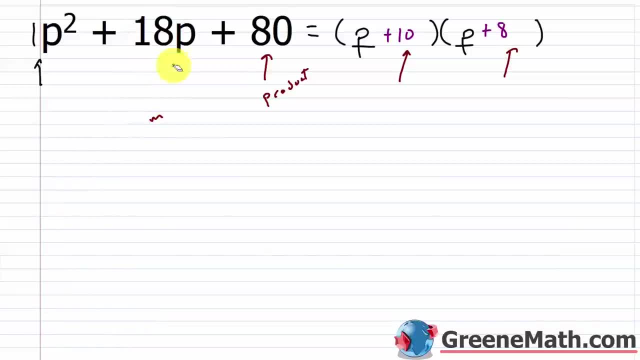 like to check things. those of you who watch my videos know that, so let's spend a little bit of time here and just check it. so if I have p times p, that's p squared, then p times 8, that's plus 8p, then 10 times p, that's plus. 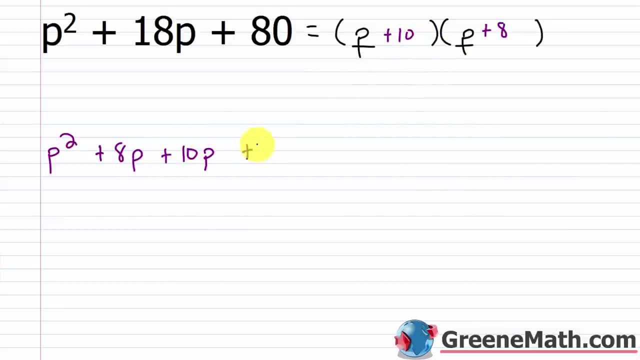 10p, and then 10 times 8, that's plus 80, and you can see that these two middle terms, the sum is going to be this right here: 18p. that's what you're looking for. this number plus this number gives you this number. 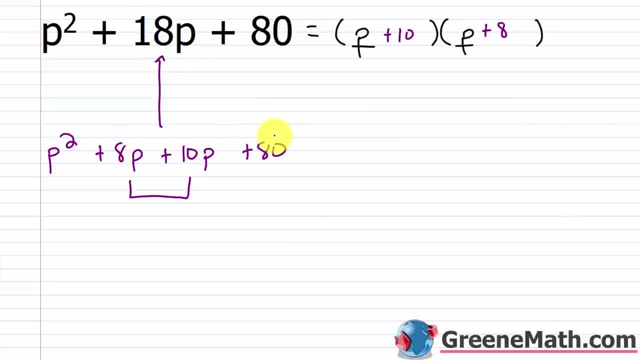 this number times this number gives you this number. so again, two integers whose sum is b, whose product is c. alright, let's take a look at another one. so we have p squared minus 11p plus 28. so again, I don't have anything to factor out of here. that's a. 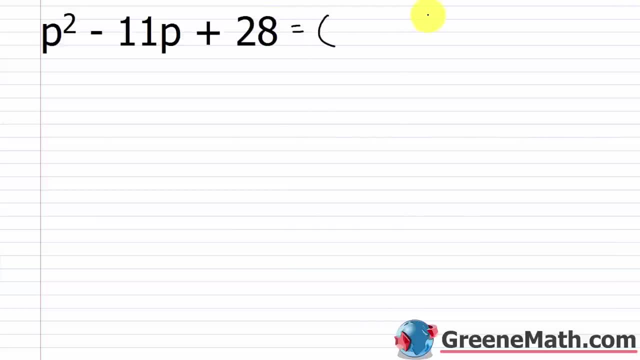 common factor to start. so I'm just going to go ahead and write my parentheses, and I know what goes. in the first position of each I have p squared. so that means I have a p here and a p here, p times p is p squared. now for this part, right here. 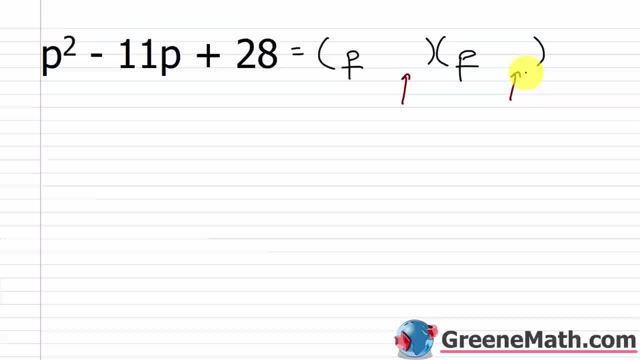 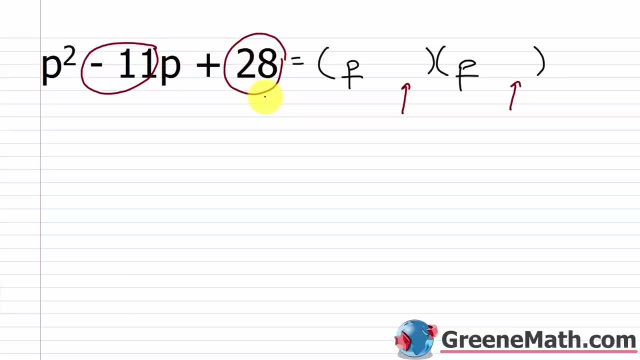 I need two integers whose sum is now negative 11, and whose product is positive 28. so because we have a negative involved, it's a little bit more complicated, because now not only do we have to think about the factors of 28, we also have to play. 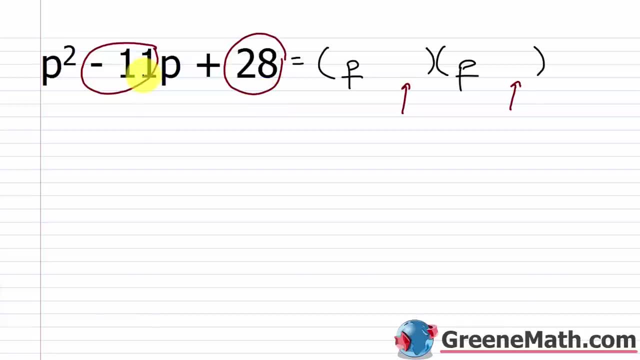 around with the signs to get the addition and the multiplication to work out. so let's just think about the factors of 28. so we have 1 and 28. those are too far apart to ever produce negative 11. no matter what the signs are, we'd have 2. 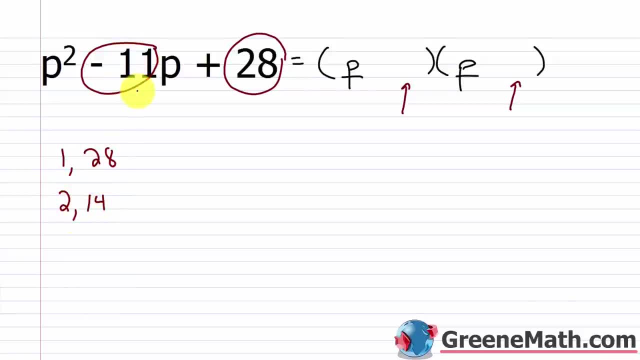 and 14. if I did 14 minus 2, that would give me 12, so that's not going to work. and if I did 2 plus 8 is 10, so it's not divisible by 3, it is divisible by 4. I can do. 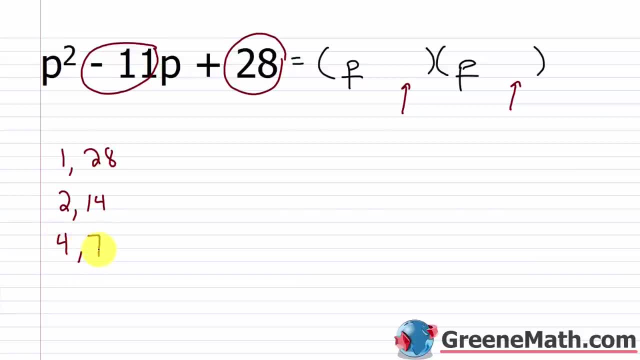 4 and 7. looks like that might work if I had a negative 4 and a negative 7. negative 4 plus negative 7 is negative 11. right sign is the same. keep the sign the same and you just add absolute values. so I would have. 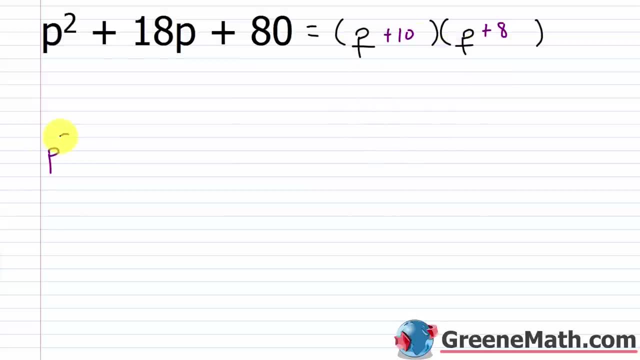 So if I have p times p, that's p squared. Then p times 8, that's plus 8p. Then 10 times p, that's plus 10p. And then 10 times 8, that's plus 80. 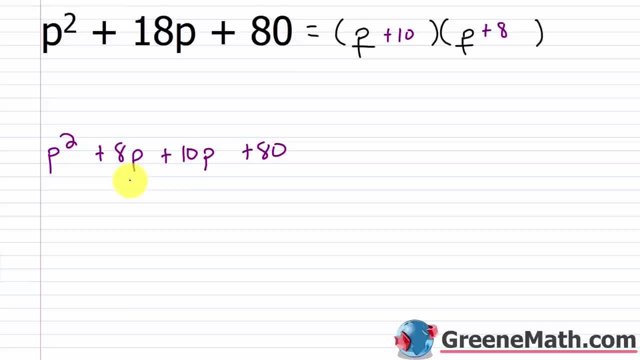 And you can see that these two middle terms, the sum is going to be this right here, 18p. That's what you're looking for. This number plus this number gives you this number. This number times this number gives you this number. 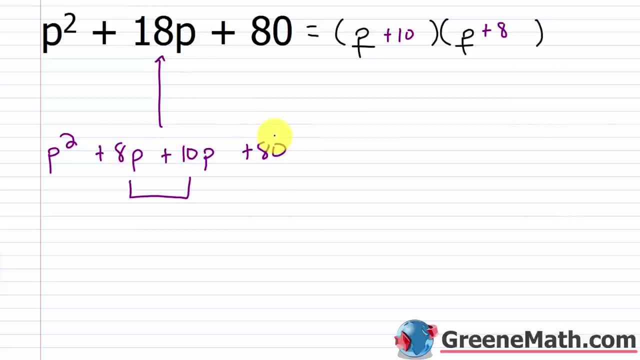 So again, two integers whose sum is b, whose product is c. All right, let's take a look at another one. 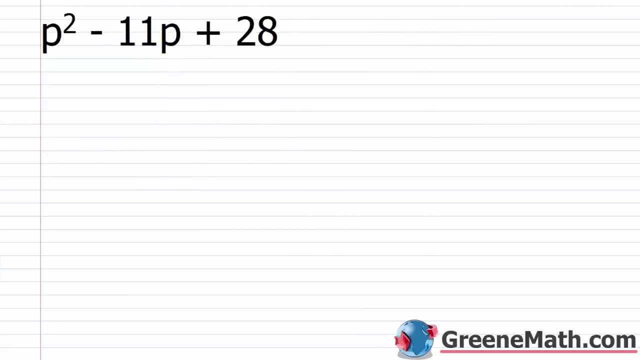 So we have p squared minus 11p plus 28. 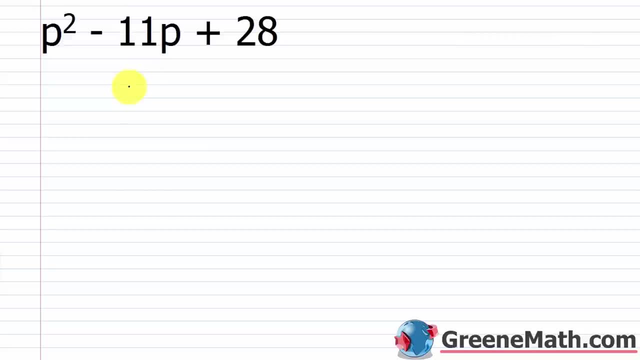 So we have p squared minus 11p plus 28. 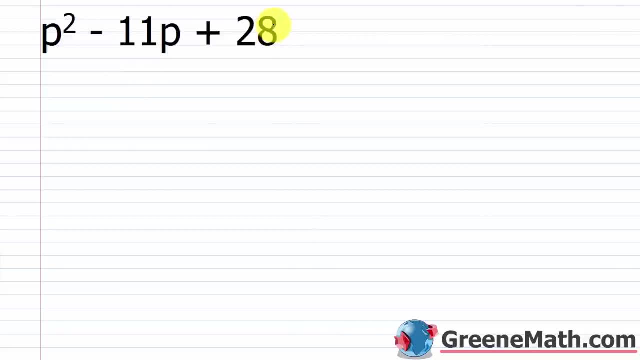 So again, I don't have anything to factor out here that's a common factor to start. So I'm just going to go ahead and write my parentheses. And I know what goes in the first position of each. 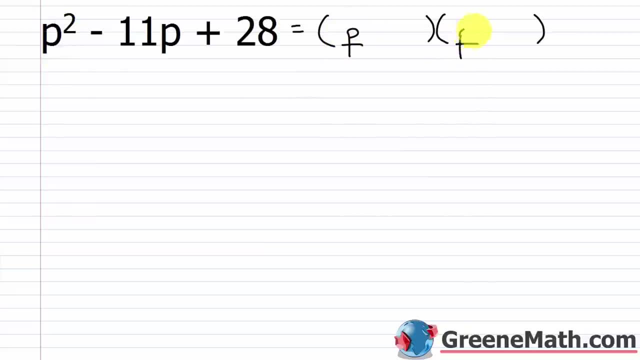 I have p squared, so that means I have a p here and a p here. p times p is p squared. 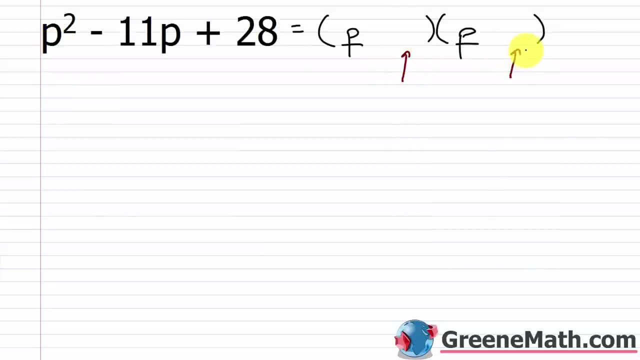 Now, for this part right here, I need two integers whose sum is now negative 11 and whose product 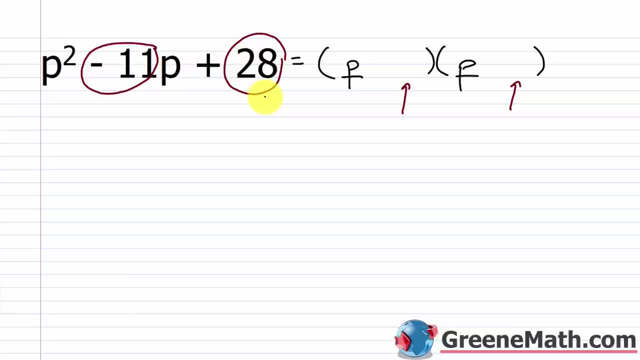 is positive 28. So because we have a negative 28 involved, it's a little bit more complicated because now not only do we have to think about the factors of 28, we also have to play around with the signs to get the addition and the multiplication to work out. 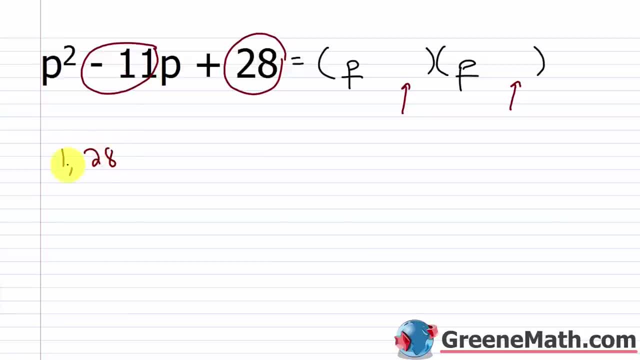 So let's just think about the factors of 28. So we have 1 and 28. Those are too 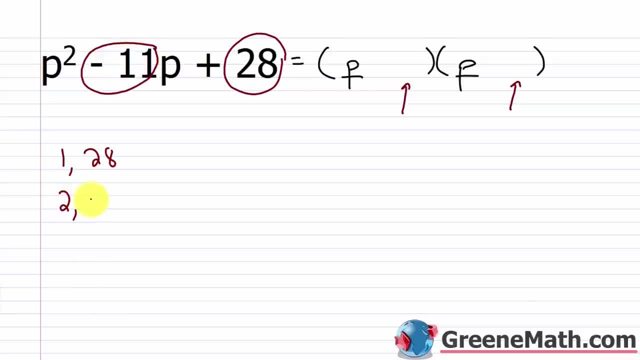 far apart to ever produce negative 11, no matter what the signs are. We'd have 2 and 14. If I did 2 plus 8 is 10, so it's not divisible by 3. It is divisible by 4. 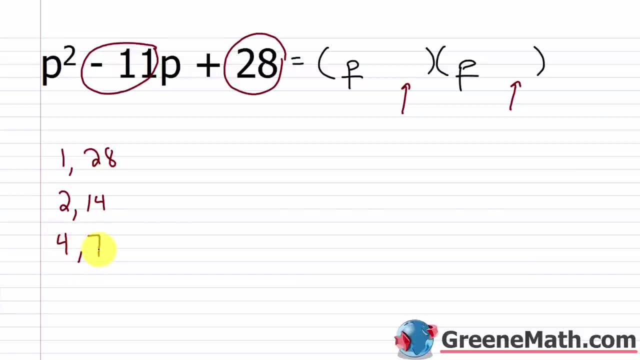 I can do 4 and 7. It looks like that might work. 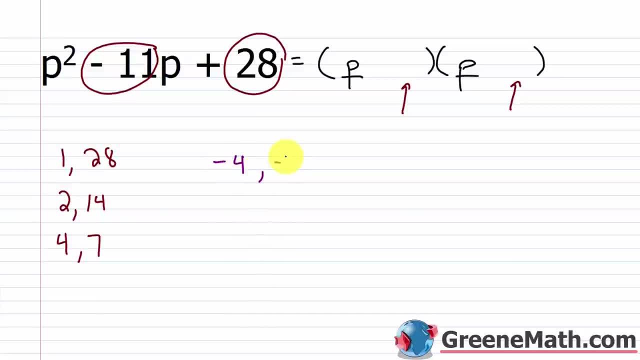 If I had a negative 4 and a negative 7, negative 4 plus negative 7 is negative 11. The sign is the same. Keep the sign And you just add absolute values. So I would have negative 11 plus 28. So that is what we're looking for. We're looking for a negative 4 and a negative 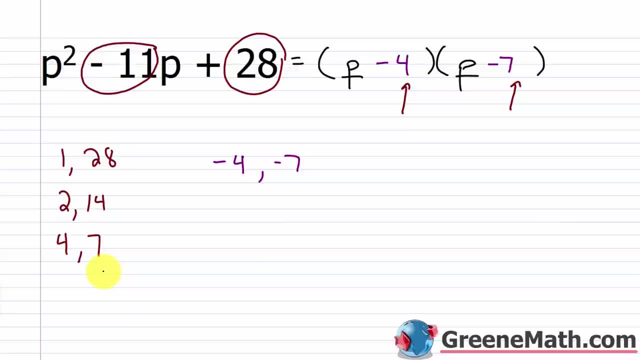 Again, once you figure out what it is, you just stop. 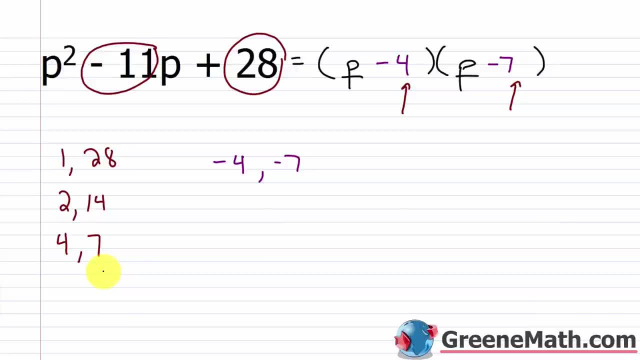 This is just you're listing a list of factors just to figure this out. 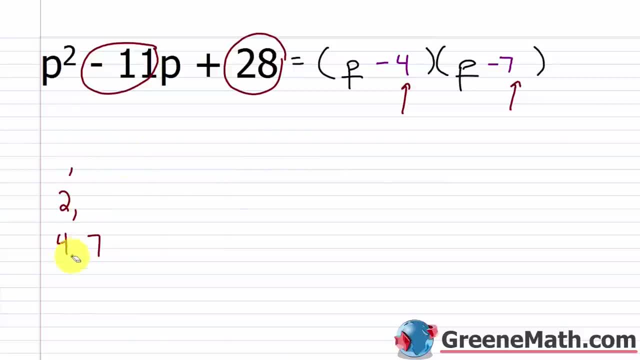 It's not like your teacher's going to grade you on, you know, 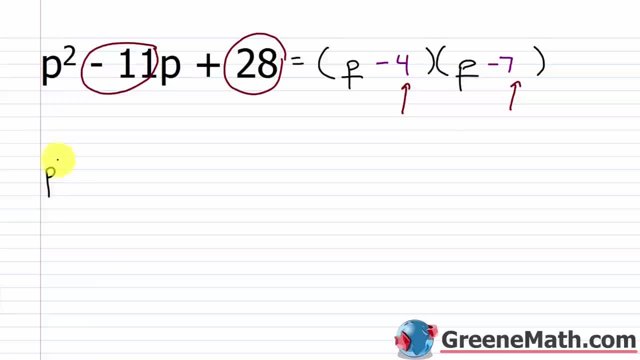 coming up with all the factors of 28. 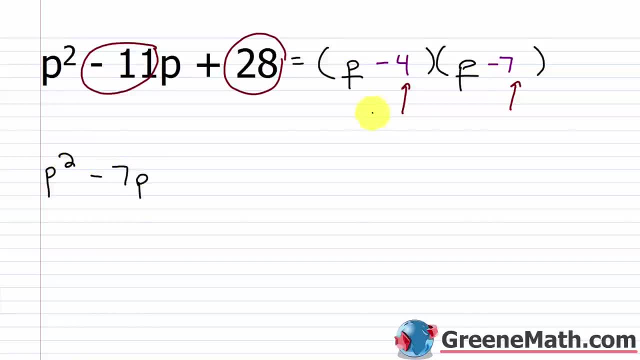 So let's go ahead and erase this. 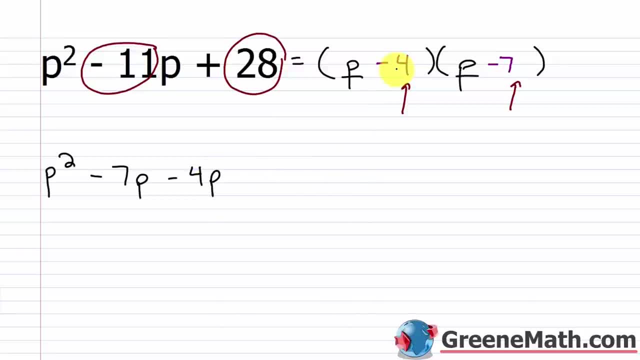 So we have negative 4 times p minus 4p. 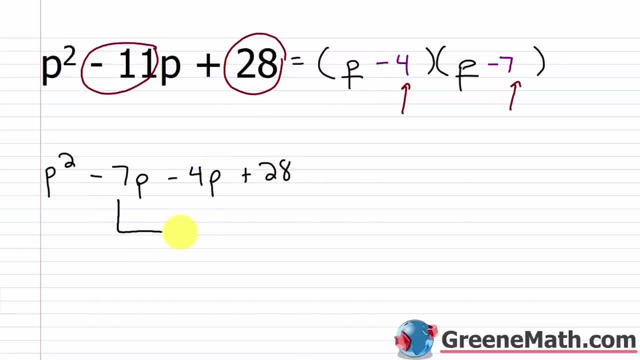 And then lastly, we have negative 4 times negative 7. That's plus 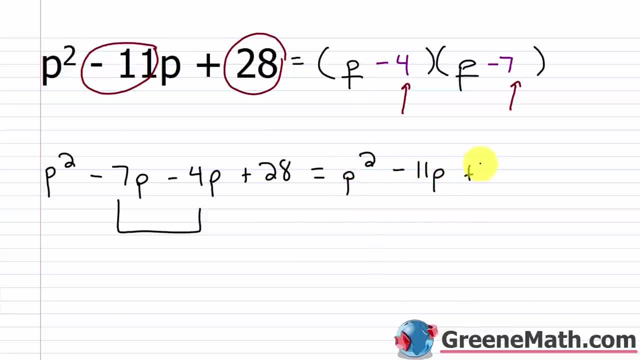 28. And again, if I combine like terms here, I would have p squared minus 11p plus 28. 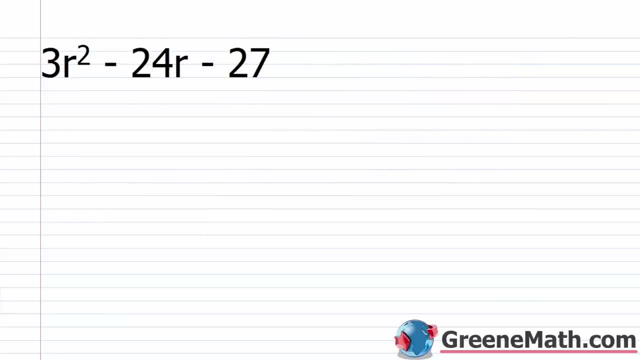 Exactly what I started with right there. 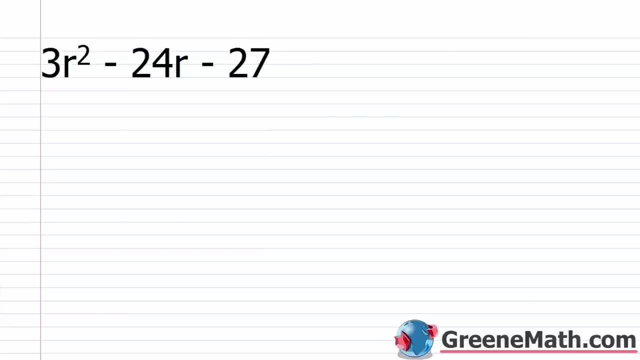 So although it's a little bit more work, a little bit more work, what you'll notice here is that everything is divisible by 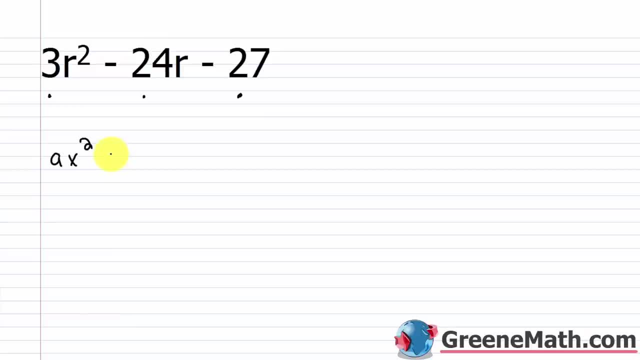 3. Because you might look at this problem and say, well, you know, if I'm looking at ax squared plus bx plus c, well, the coefficient on the 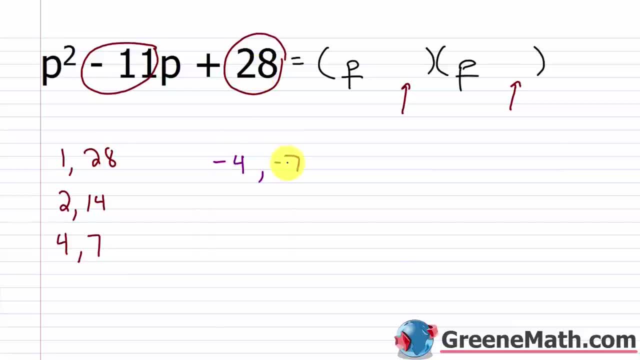 negative 11. from that, negative times negative is positive. negative 4 times negative 7 is positive 28. so that is what we're looking for. we're looking for a negative 4 and a negative 7 again. once you figure out what it is, you just stop. 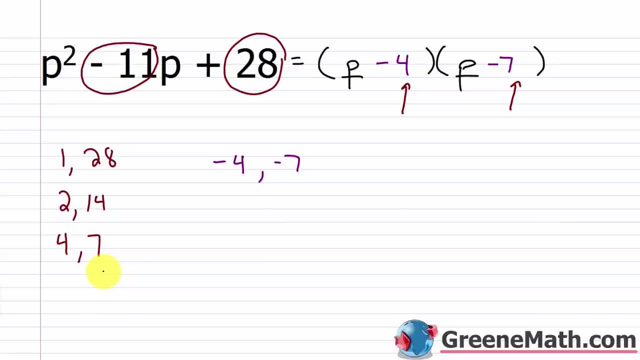 this is just you're listing a list of factors. just to figure this out. it's not like your teacher is going to grade you on. you know coming up with all the factors of 28, so let's go ahead and erase this and we can check our results. 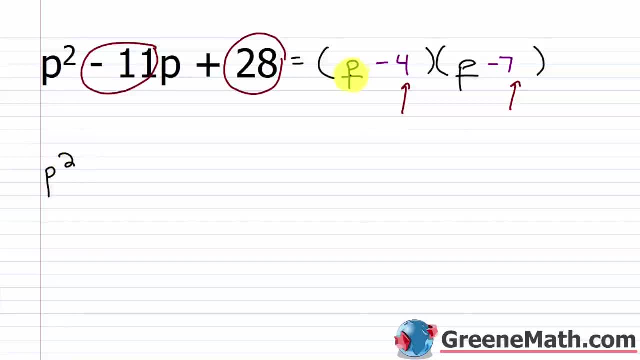 so p times p is p squared. the outer p times negative 7 is negative 7p, the inner negative 4 times p is minus 4p. and then lastly, we have negative 4 times negative 7, that's plus 28, and again, if I 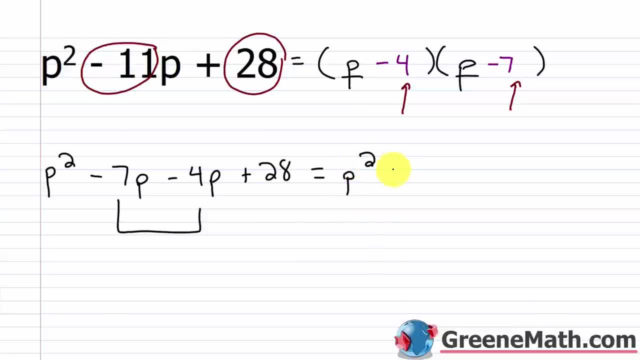 combine like terms here, I would have p squared minus 11p plus 28- exactly what I started with right there. so although it's a little bit more work, a little bit more complex if you have a negative sign involved, it's still pretty easy overall. alright, let's take a look at. 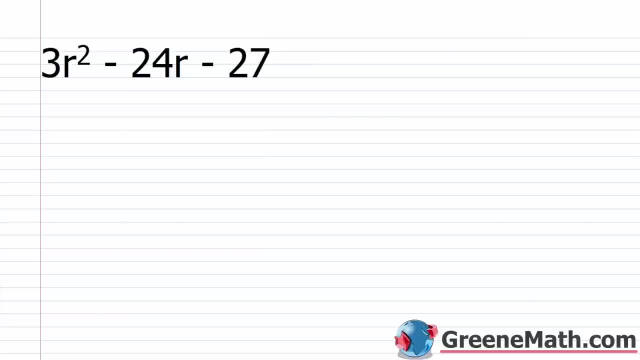 3r squared minus 24r minus 27. so one thing you'll notice here is that everything is divisible by 3, because you might look at this problem and say: well, you know, if I'm looking at ax squared plus bx plus c, well, the coefficient. 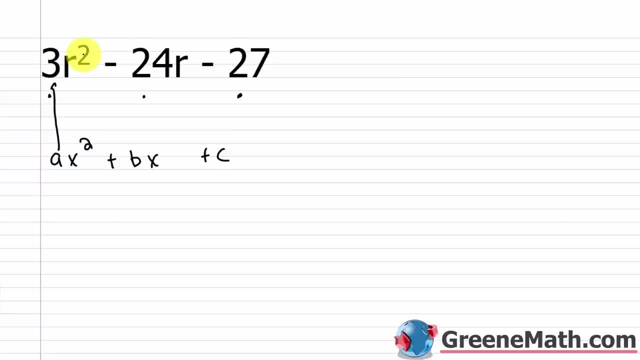 on the squared term. here it's r. doesn't matter if it's r or z or q, whatever it is. the coefficient on the variable that's squared is not 1 here. so if you're in a section where the coefficient is supposed to be 1, 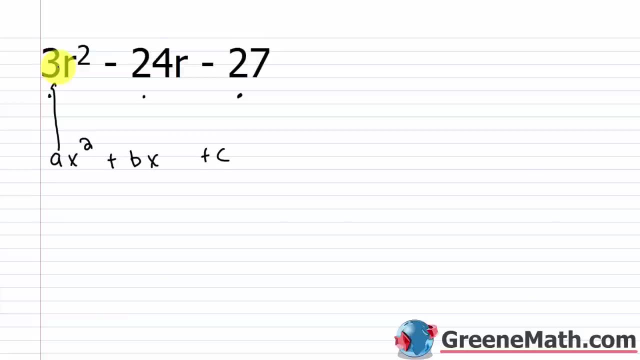 that should clue you in that. hey, I need to do some additional work before I can start and you can see that everything is divisible by 3, so we're going to pull that out. so I'm going to put a 3 out in front, inside the parentheses. 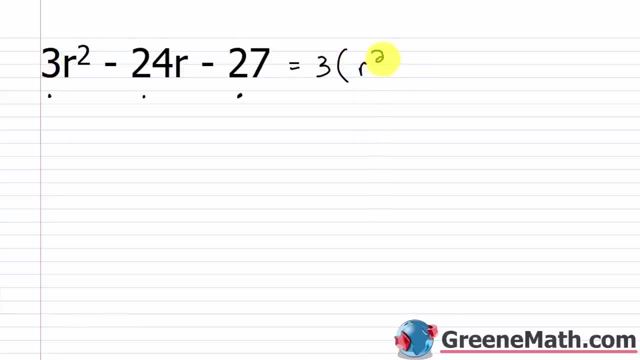 I'm going to have 3r squared divided by 3, that's r squared, negative 24r divided by 3, that's minus 8r negative 27 divided by 3 is negative 9. I'm just going to think about what's inside the 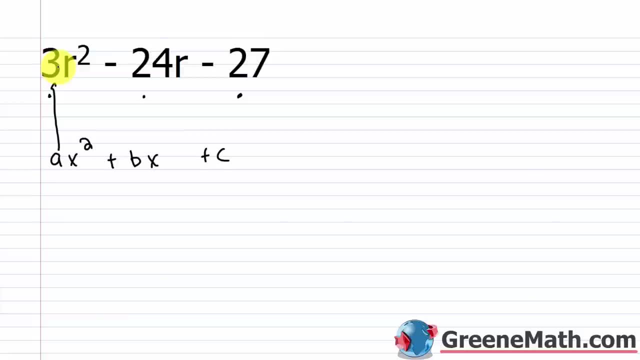 squared term here, it's r, doesn't matter if it's r, z, or q, whatever it is, and you can see that everything is divisible by 3. So we're going to pull that out. So I'm going to put a 3 out in front. 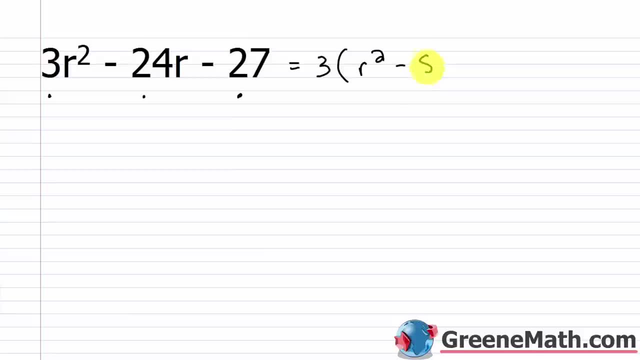 Inside the parentheses, I'm going to have 3r squared divided by 3, that's r squared, negative 24r 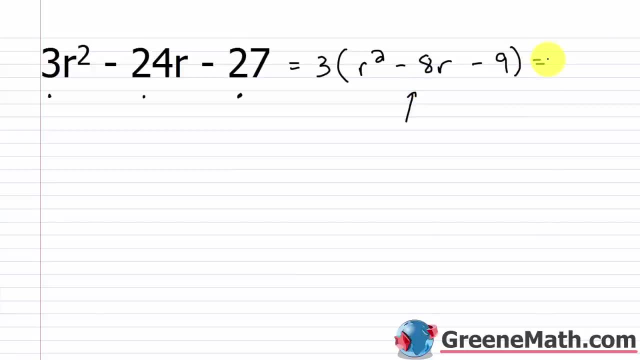 divided by 3, that's minus 8r, negative 27 divided by 3 is negative 9. 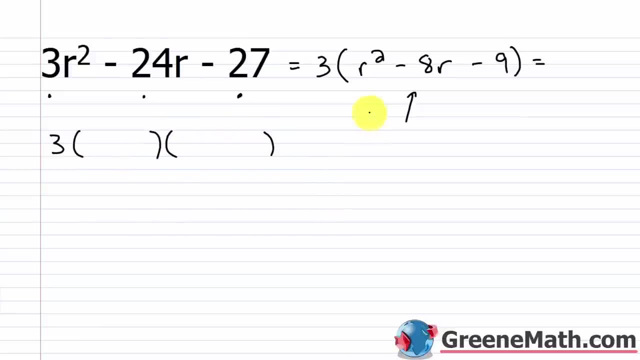 So I'm going to put r in the parentheses, and then another set of parentheses. So nothing has changed. r squared here, 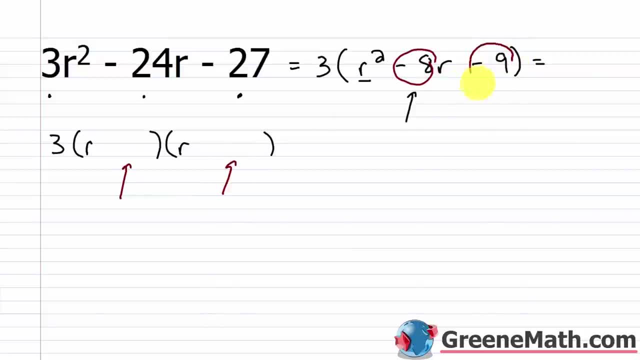 I'm going to put r, and then r. 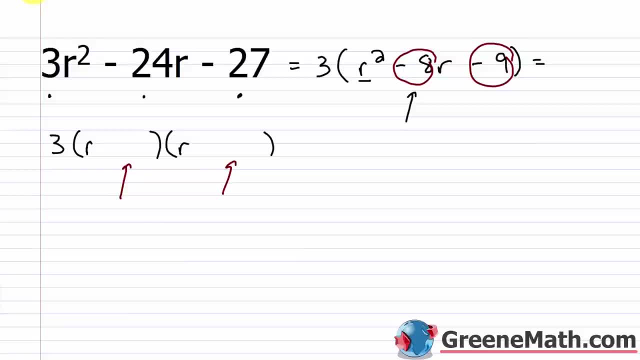 And now I need two integers whose sum is now negative 8, and whose product is negative 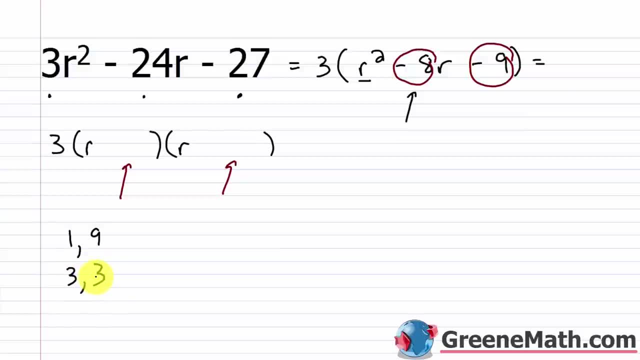 Well, it can't be 3 and 3 because there's no combination that's going to get you a sum of negative 8. 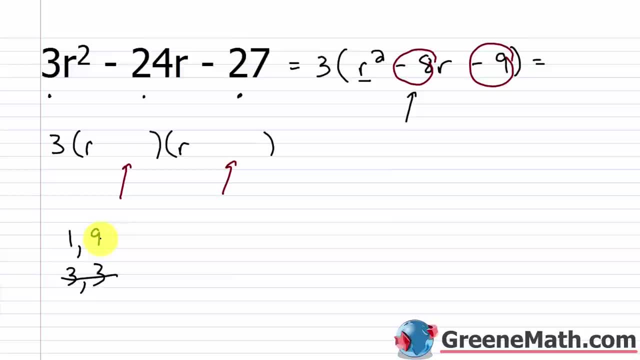 It doesn't matter how you play with the signs. So that's 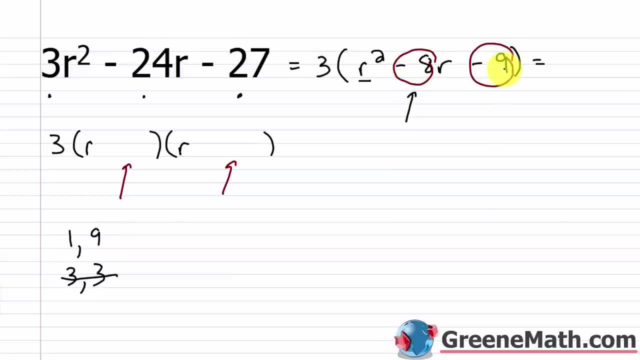 So I need to play with 1 and 9. 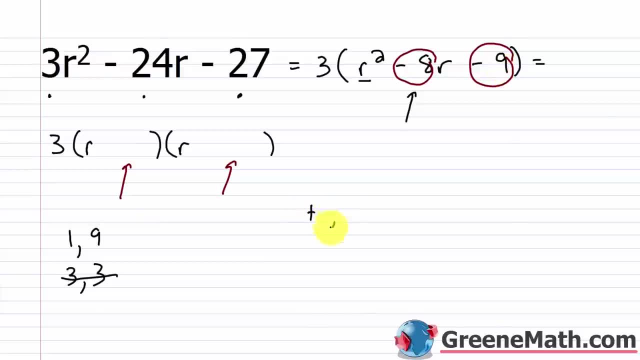 Now I know that the middle term is negative, and the last term is negative. I can only get that if I have 1 and 9. 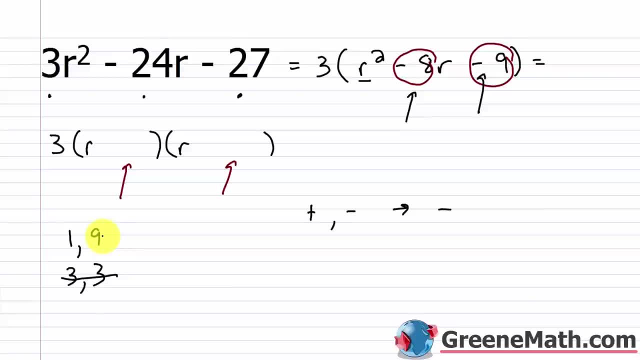 Now we think about the fact that we have 1 and 9. Which one would I make negative? Which one would I make positive? Well, obviously 9 would 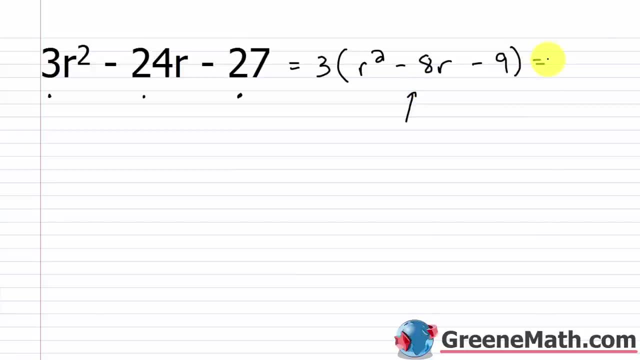 parentheses here. so when I set up my kind of two binomials, I'm going to get 3 times. we'll have a set of parentheses and then another set of parentheses. so nothing has changed. r squared here. I'm going to put r and then r. 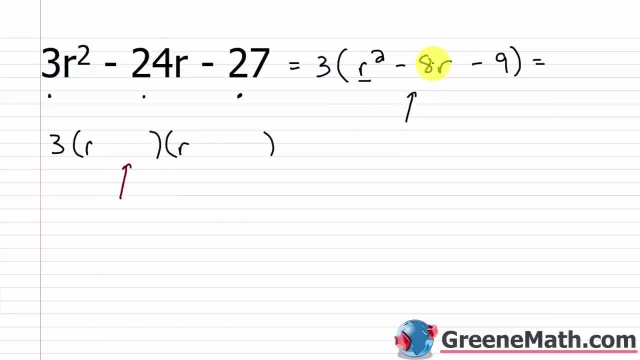 and now I need two integers whose sum is now negative 8 and whose product is negative 9, two integers that fit that profile. so let's think about factors of just 9, forget about the fact that it's negative, just factors of 9. you've got 1 and 9. 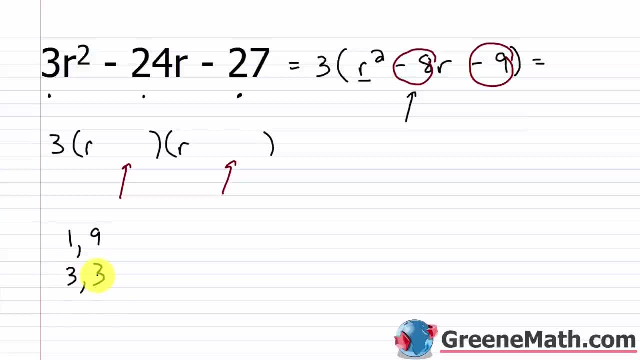 and you've got 3 and 3. well, it can't be 3 and 3 because there's no combination. that's going to get you a sum of negative 8. it doesn't matter how you play with the signs, so that's out. so I need to play with 1. 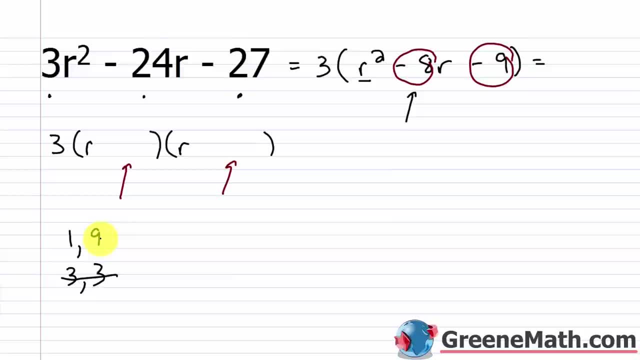 and 9. now I know that the middle term is negative and the last term is negative. I can only get that if I have different signs right, because we know that a positive times a negative will yield us a negative. so that's how we got that: through multiplication. 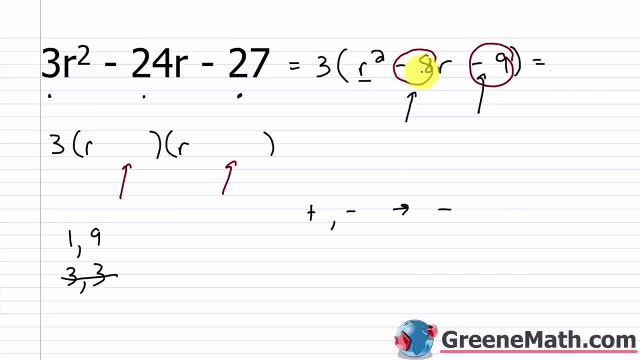 so 1 is positive, 1 is negative. now we think about the fact that we have 1 and 9. which one would I make negative? which one would I make positive? well, obviously 9 would become negative. I put negative 9 and positive 1 and that would get us. 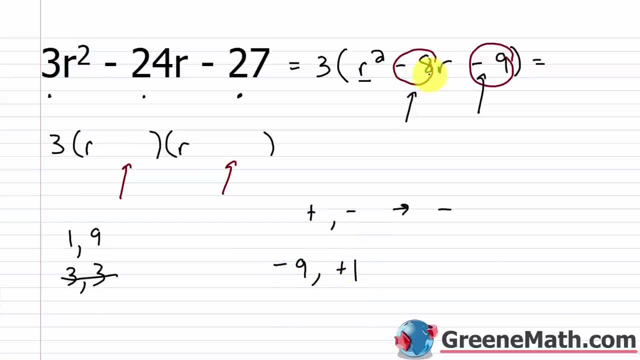 exactly what we need. negative 9 plus 1 would give us negative 8. negative 9 times 1 would give us negative 9. so we're good to go there. so my integers would be negative 9. so I put minus 9 and positive 1. 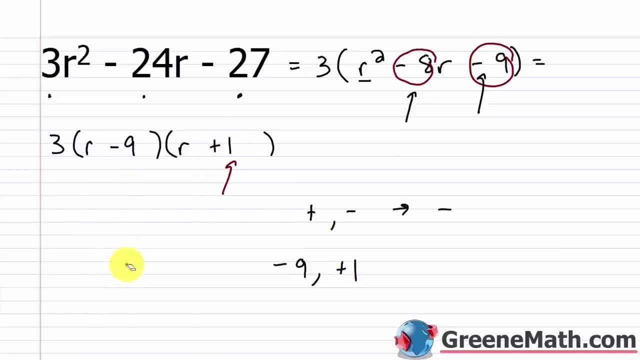 so I put plus 1, and again I like to check things. so let's erase all this and let's do r times r, that's r squared, and then r times 1, that's plus r negative. 9 times r, that's minus 9r. 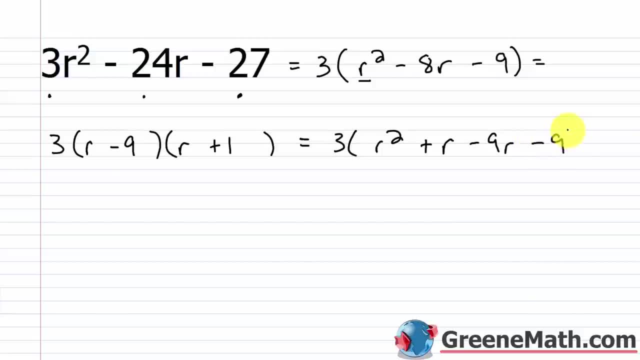 and then negative 9 times 1, that's minus 9. if I combine like terms in the middle, I will have 3 times r? squared minus 8r minus 9. and then, if I continue, I just multiply: 3 times r squared, that's 3r squared. 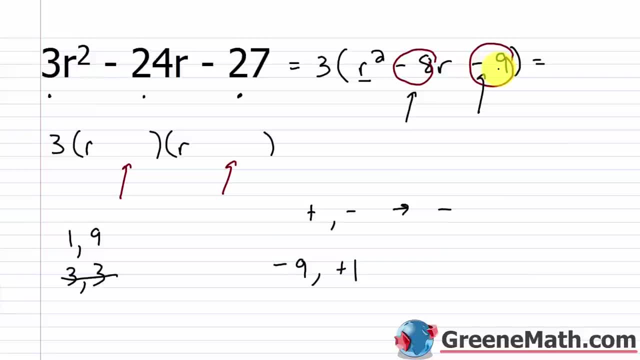 become negative, right? I put negative 9 and positive 1, and that would get us exactly the same thing. 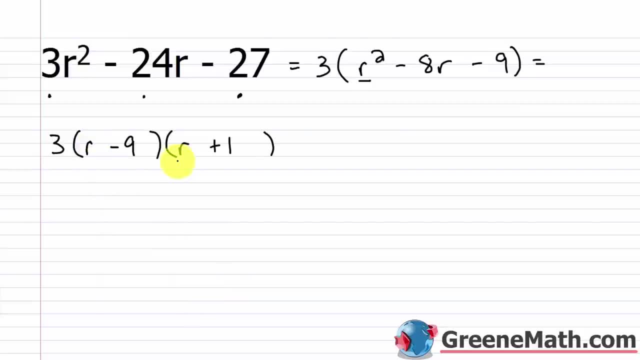 So let's erase all this, and let's do r times r, that's r squared, and then r times 1, that's plus r, negative 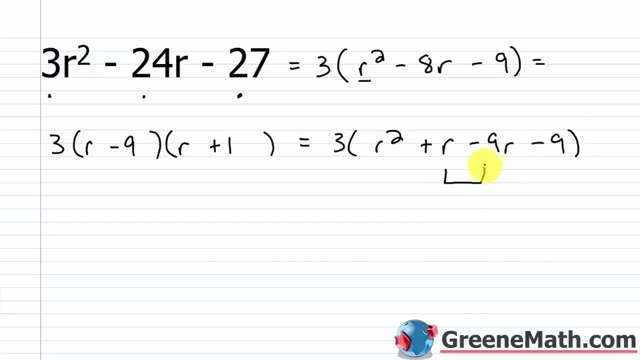 9 times r, that's minus 9r, and then negative 9 times 1, that's minus 9. 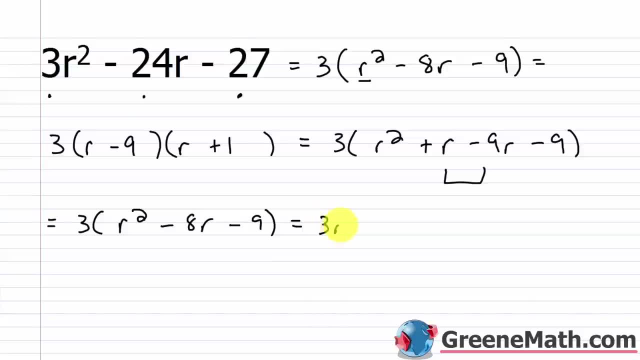 If I continue, I just multiply 3 times r squared, that's 3r squared, 3 times negative 8r, that's negative 24r, and then 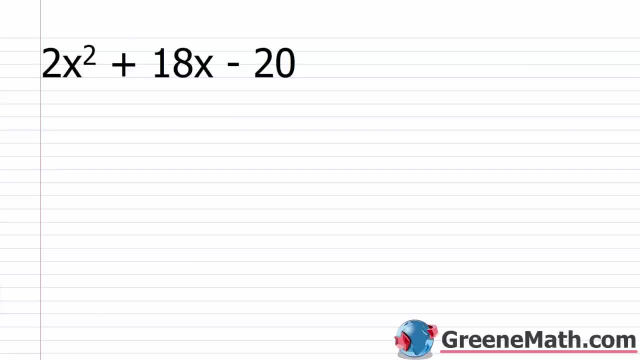 3 times negative 9 is minus 27. 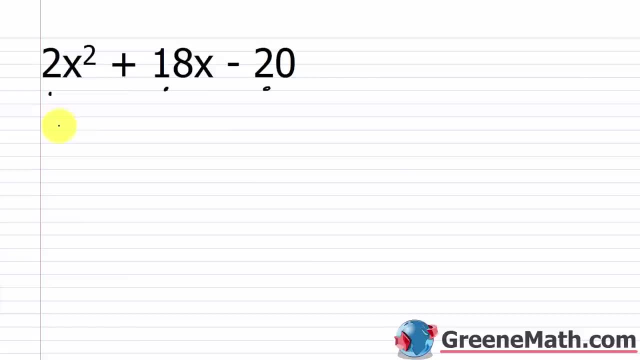 Again, that's exactly what we started with right there. 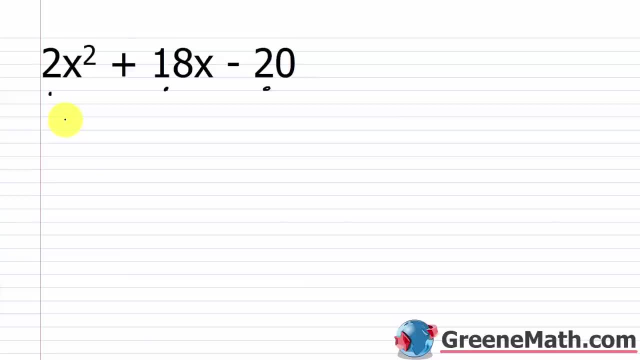 All right, so we're going to do something first, right? 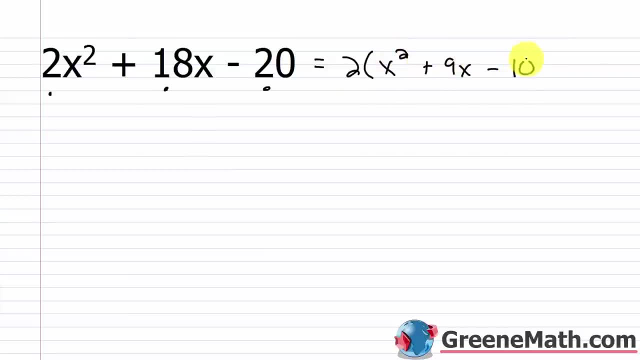 So I know that everything's divisible by 2, 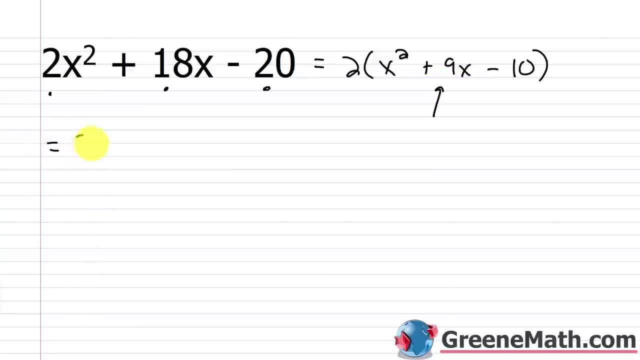 I can pull that out, and in my parentheses, I'll have x squared plus 9x minus 10. 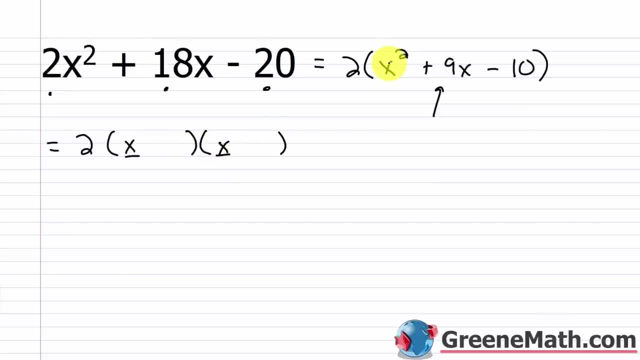 Now, I'm going to multiply this by x squared times x squared. 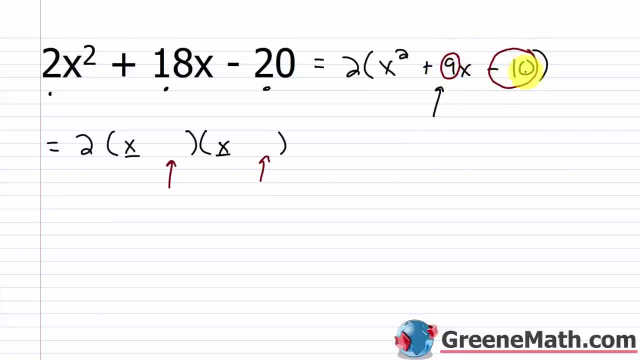 Now, how do I get these two middle terms? 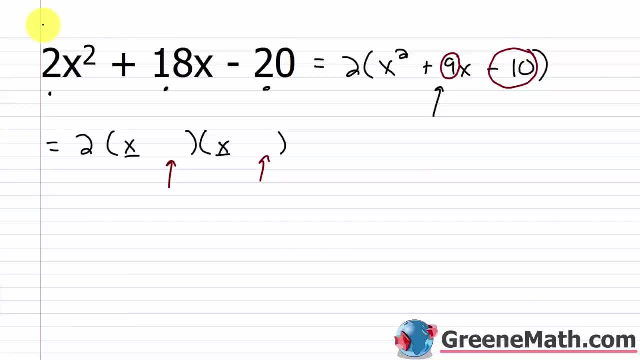 Again, two integers whose sum is 9, whose 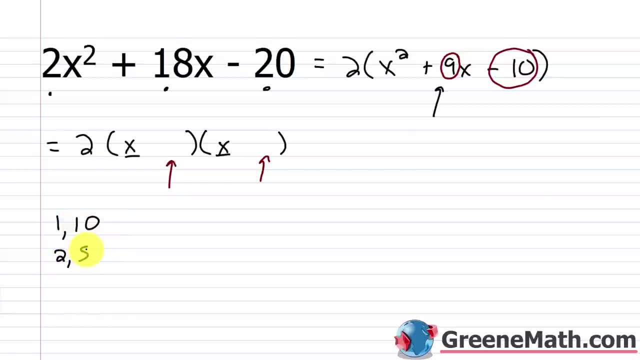 product is negative 10. 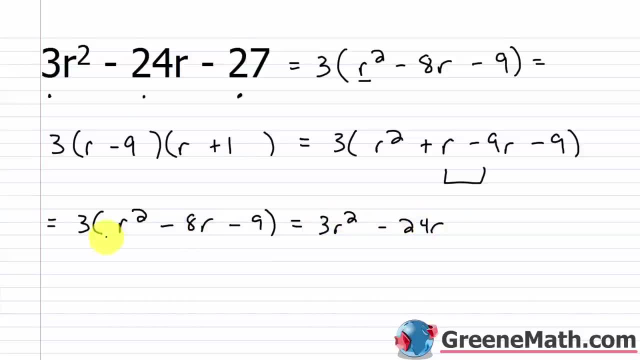 3 times negative 8r, that's negative 24r. and then 3 times negative 8r minus 27, and again, that's exactly what we started with, right there? alright, let's take a look at another one. we have 2x squared plus 18x minus 20. 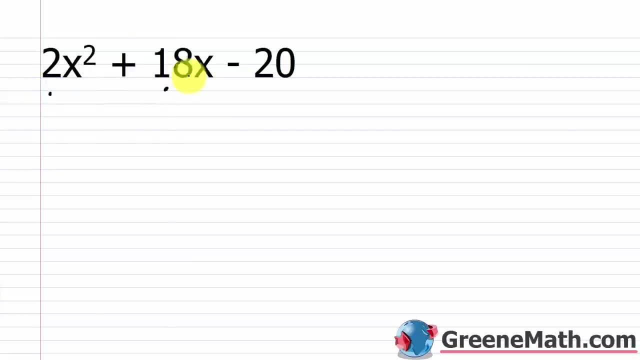 again. the first thing you should look at is: ok, all these numbers are even and the coefficient for the squared term is not a 1. so again, that's a dead giveaway, if you're in this section, where the leading coefficient is supposed to be 1, that you gotta do something first. 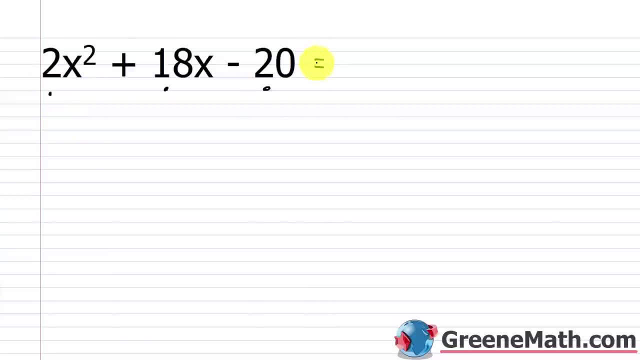 right. so I know that everything is divisible by 2. I can pull that out in parentheses. I'll have x squared plus 9x minus 10. now I'm gonna factor what's inside the parentheses here, so let's go ahead and set this up as 2 times. 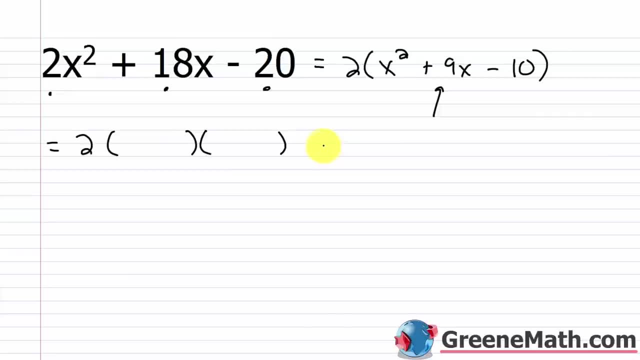 we'll put our parentheses for the 2 binomials and I know that in this position and this position, I have x squared, so it's gonna be x times x. alright, x times x is x squared. now how do I get these 2 middle terms again? 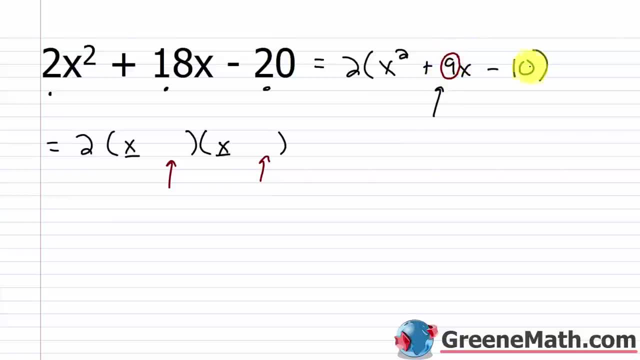 2 integers, whose sum is 9, whose product is negative 10, and again we have a negative involved. so it's a little bit more complex. just think about the factors of positive 10. forget about the negative, for right now the factors of 10. you have 1 times 10. 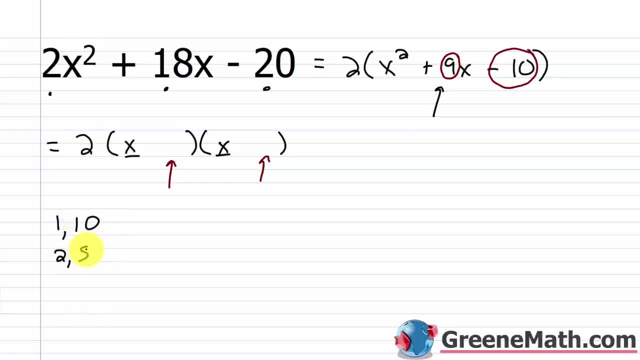 you have 2 times 5 not divisible by 3, 4, 6, 7, 8 or 9, so we can stop there. so obviously 2 and 5 are not gonna work right. there's no combination with the signs that would get you to. 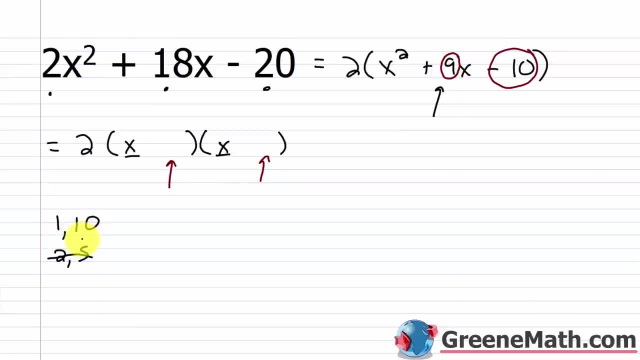 a sum of 9. what about 1 and 10? well, if I had a positive 10 and I had a negative 1, that would work. positive 10 plus negative 1 gives me a positive 9. positive 10 times negative 1 gives me a negative 10. 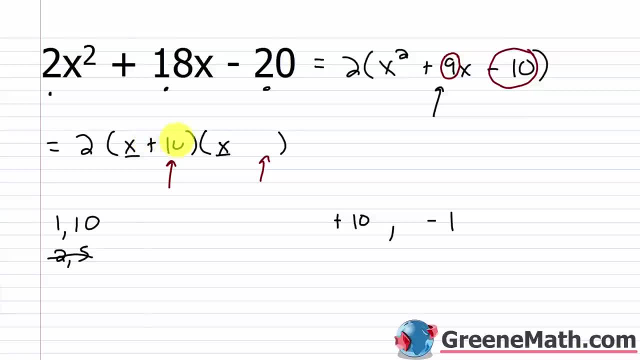 so I found my 2 integers, so plus 10 and then minus 1, very, very easy. and again, I like to check things, so let's go ahead and do: 2 times x times x is x squared outer. x times negative: 1 is minus x. 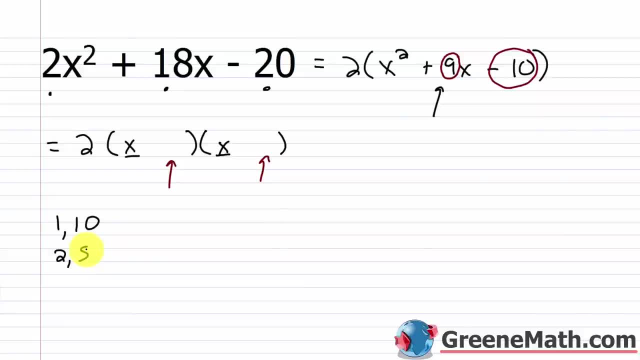 Again, we have 2 and 5. 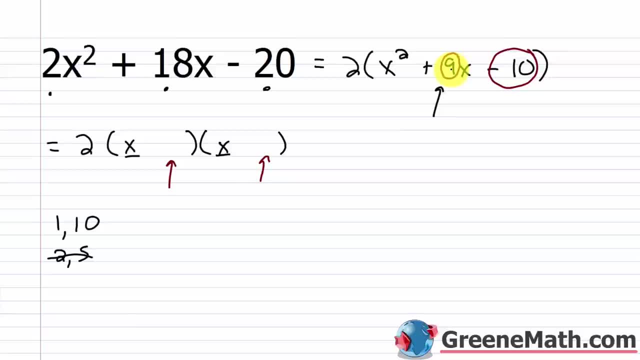 So obviously, 2 and 5 are not going to work, right? 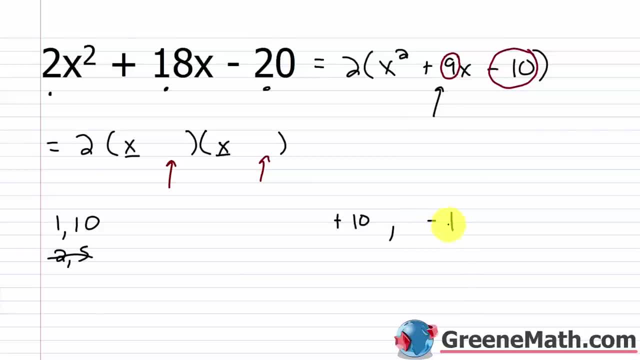 There's no combination with the signs that 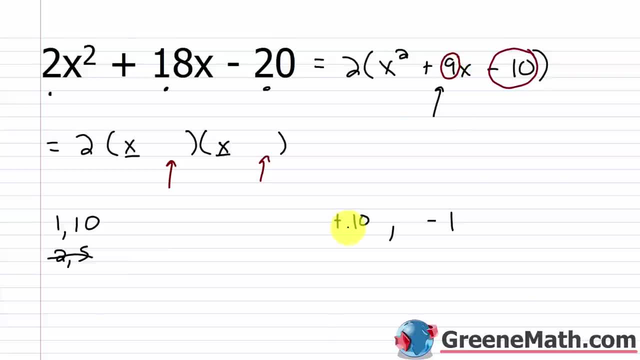 would get you to a sum of 9. 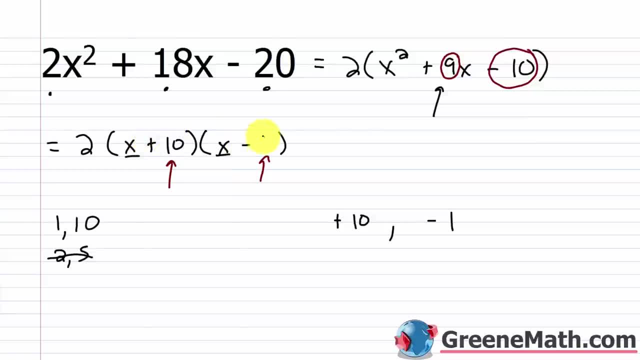 What about 1 and 10? Well, if you 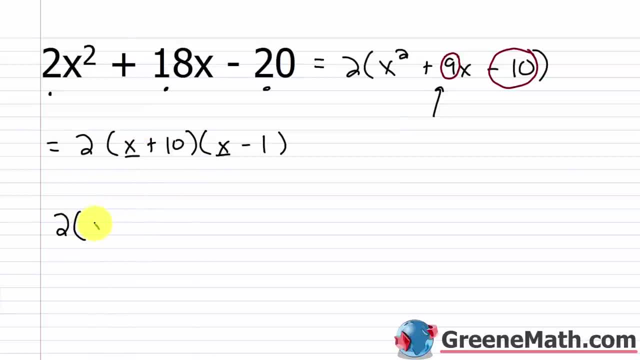 multiply this by x squared, you get 10 times x plus 10x. 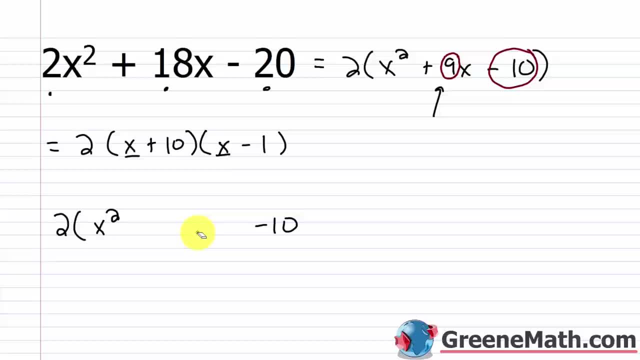 If I combine like terms here, I'd have plus 9x. 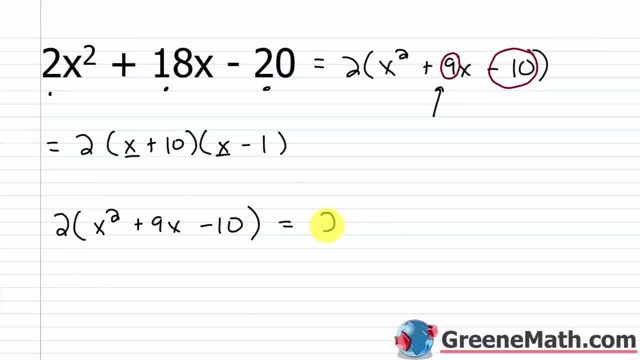 And if I multiply here, 2x squared, 2 times plus 9x is plus 18x, and then 2 times negative 10 is minus 20. 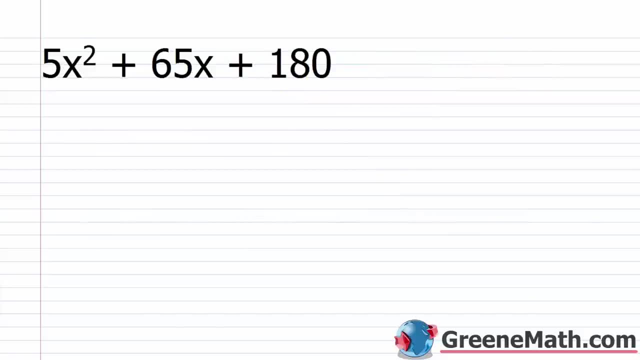 So 2x squared plus 18x minus 20. 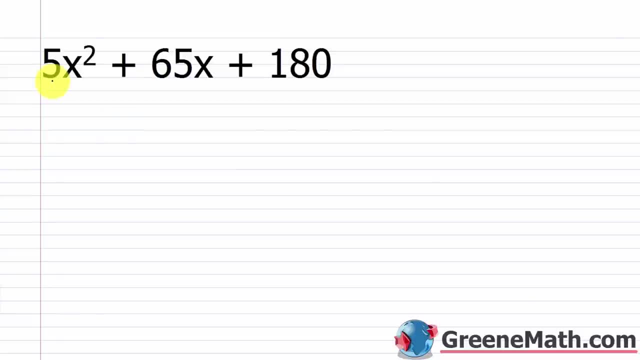 And that's exactly what we started with. 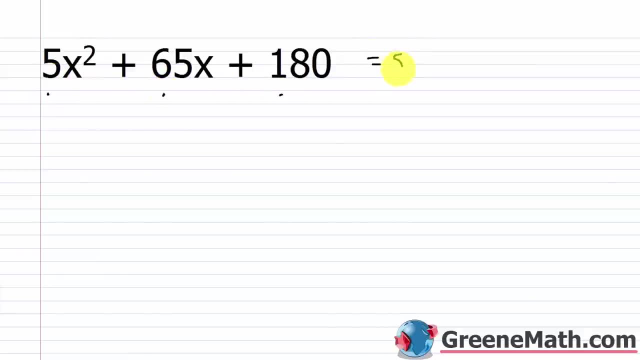 All right, for the next one, I'd have x squared plus 13x plus 36. 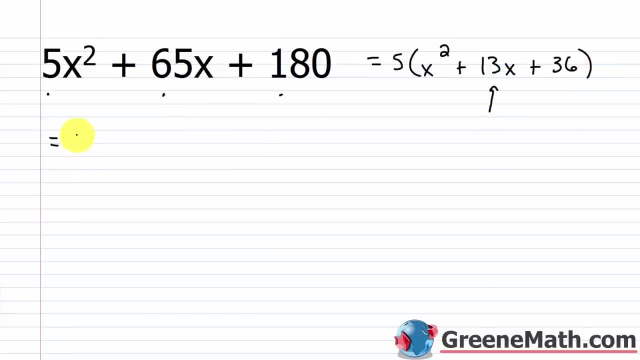 All right, so now I'm going to factor what's inside the parentheses here. 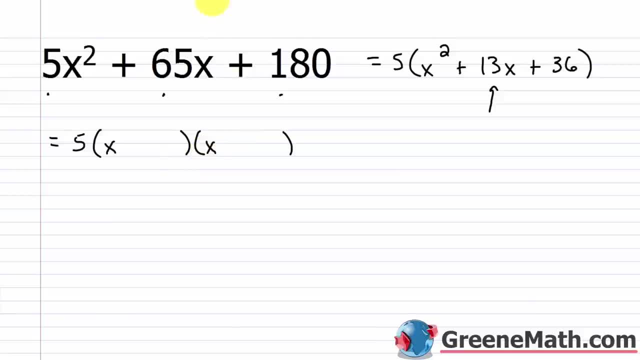 So let's go ahead and write this as equals 5 times. 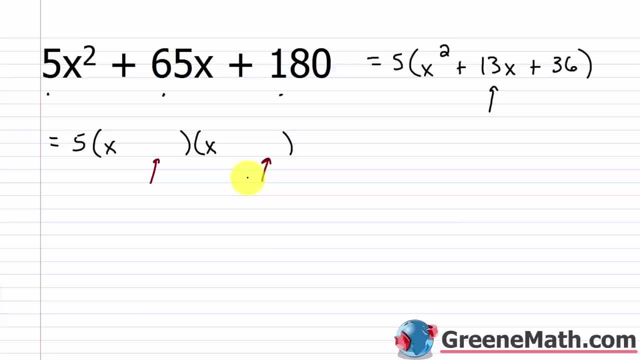 We'll put the answer in the next one. 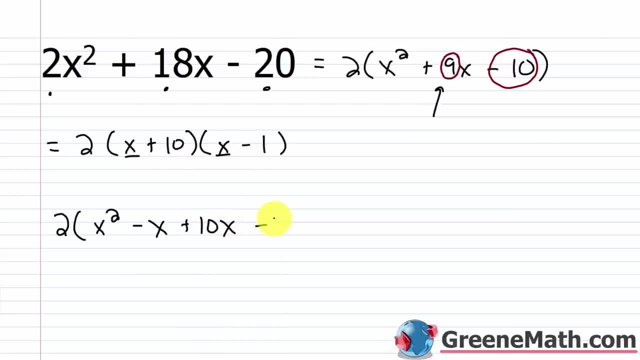 1 times x is plus 10x, and then 10 times negative 1 is minus 10. if I combine like terms here, I'd have plus 9x. let me scooch this down a little bit. and if I multiply here, I'd have 2 times x squared. 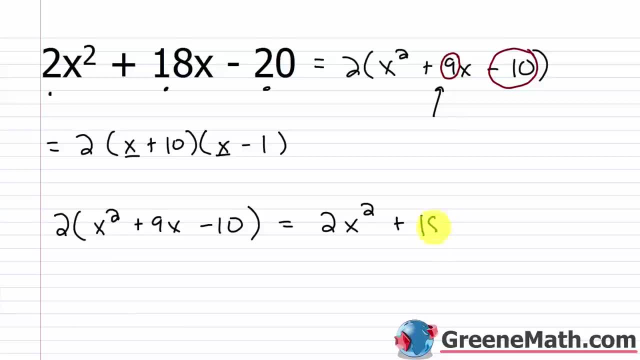 that's 2x squared, 2 times plus 9x is plus 18x, and then 2 times negative: 10 is minus 20. so 2x squared plus 18x minus 20, and that's exactly what we started with. alright, for the next one, I have 5x squared. 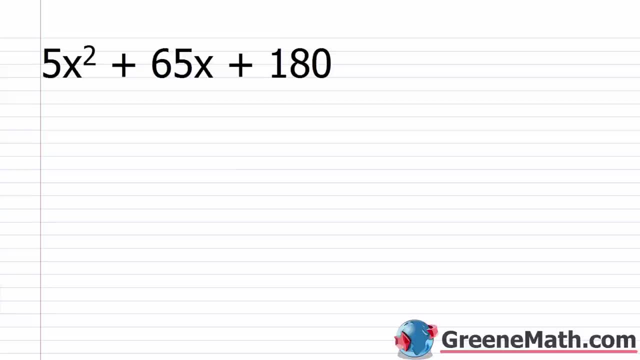 plus 65x plus 180. and again, if I am in a section where the leading coefficient is supposed to be 1 and it's not, it's a dead giveaway that I can pull something else out. everything here is divisible by 5. so if I pulled a 5 out, 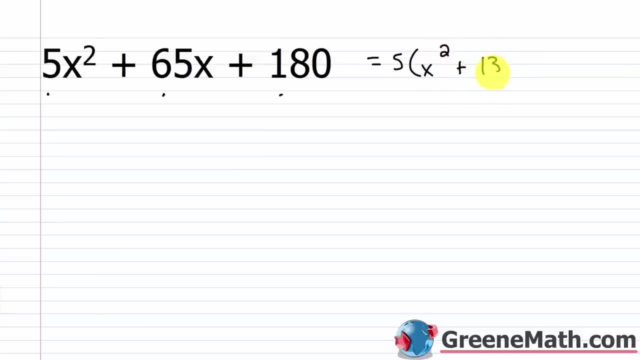 I'd have x squared plus 13x plus 36, alright, so now I'm going to factor what's inside the parentheses here, so let's go ahead and write this as equals 5 times. we'll put the parentheses for the two binomials, and I always know that if it's x squared. 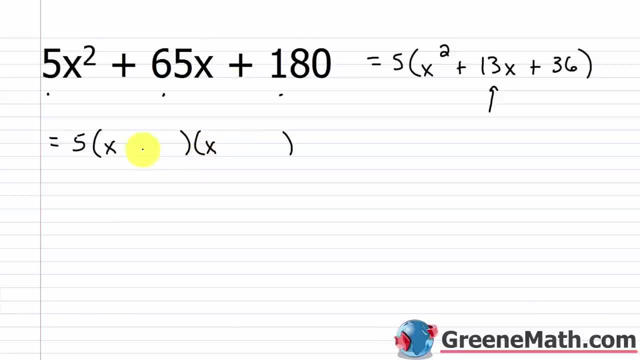 here. this will be x and this will be x. all I need to figure out is the two integers that go in those positions. so give me two integers whose sum is 13 and whose product is 36. so let's think about that. for 36, we have 1 times. 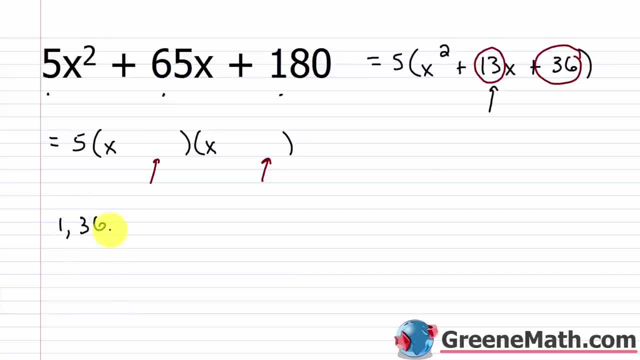 36 and obviously that's not going to work. for the next one, we could do 2 times 18. that's not going to work. we could do 3 times 12 and that's not going to work. we could do 4 times 9. 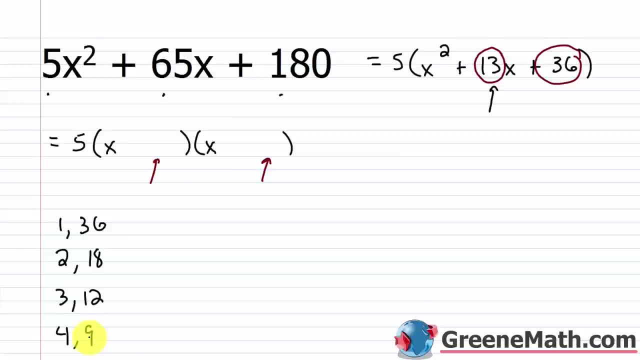 and that will work. 4 plus 9 is 13, 4 times 9 is 36. so plus 4 and plus 9, and there you go. you have 5 times the quantity x plus 4 times the quantity x plus 9. and again, if you want to check this, 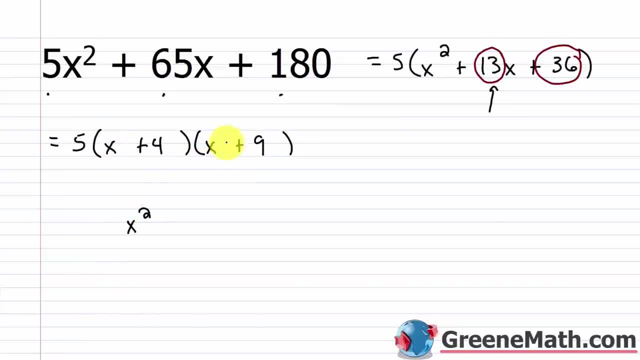 x times x is x. squared x times 9 is plus 9x. 4 times x is plus 4x. 9x plus 4x would be plus 13x, and then 4 times 9 is plus 36, and then multiply that by 5. 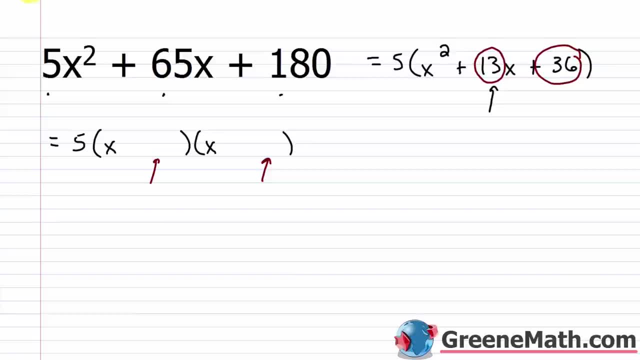 So let's think about that. 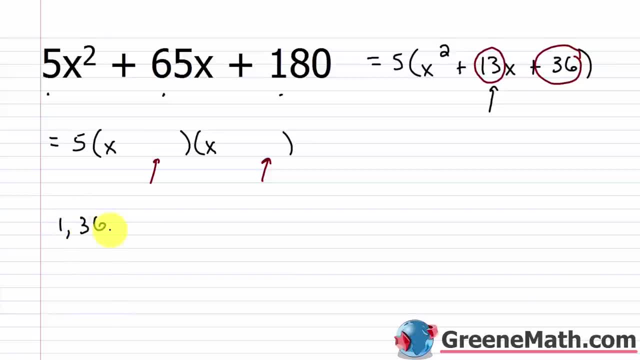 For 36, we have 1 times 36. 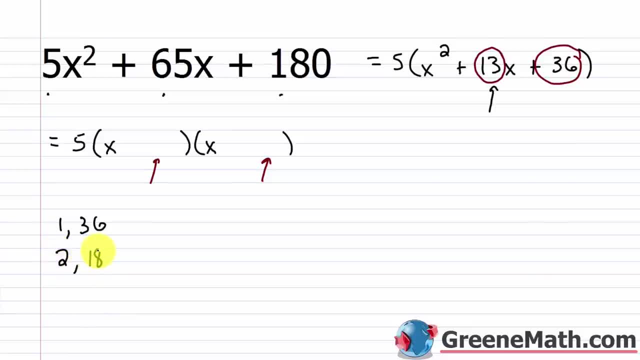 And obviously, that's not going to work. 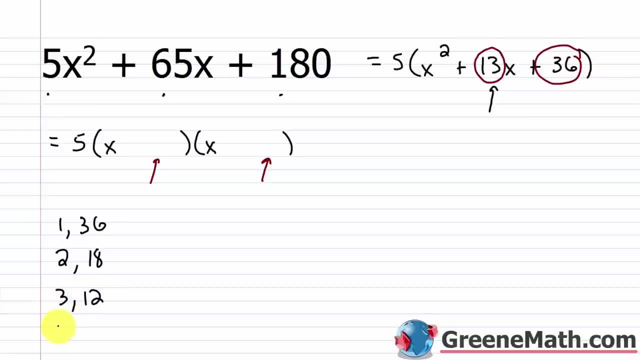 For the next one, we could do 4 times 9 is 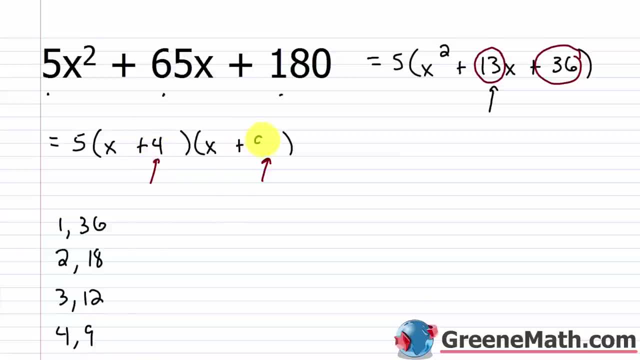 36. So plus 4 and plus 9. 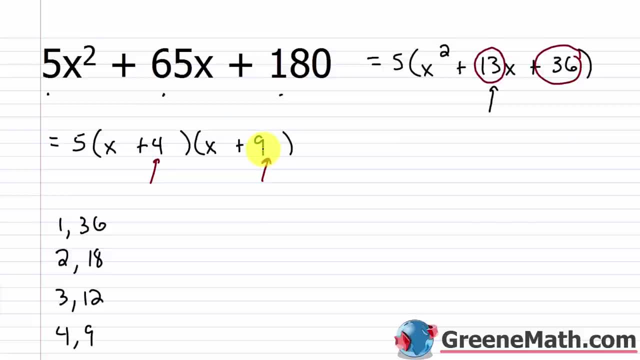 And there you go. 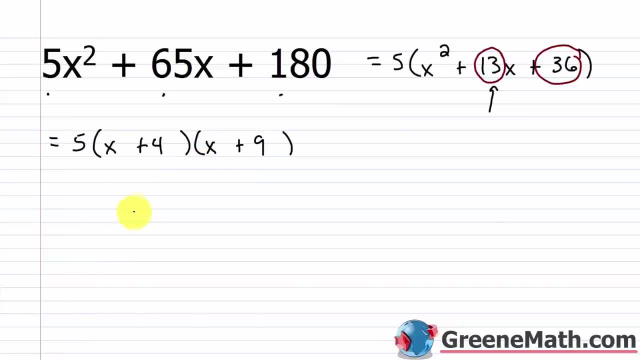 You have 5 times the quantity x plus 4 times the quantity x plus 9. 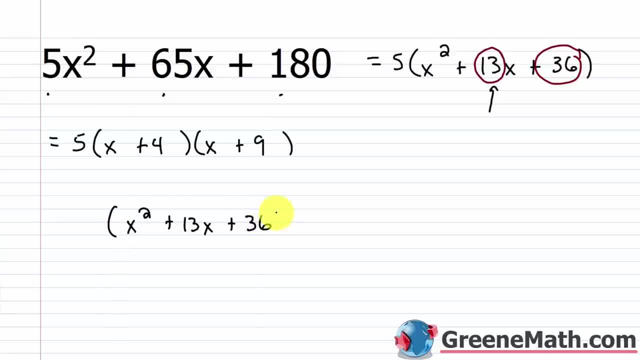 And again, if you do that, you will get this back. 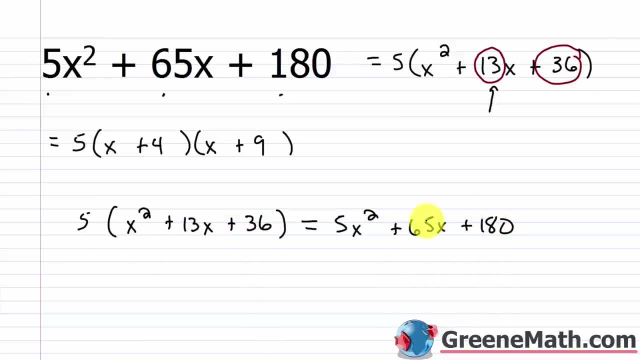 5 times x squared is 5x squared. 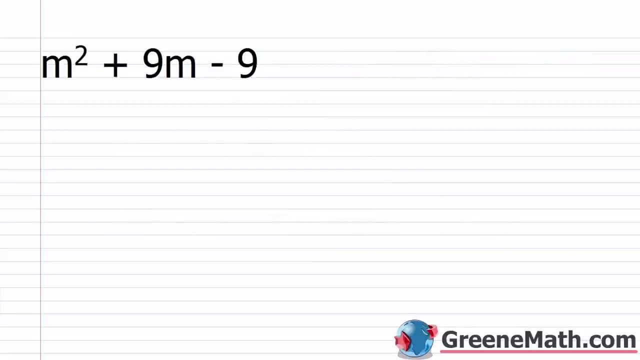 5 times 13x is plus 65x. 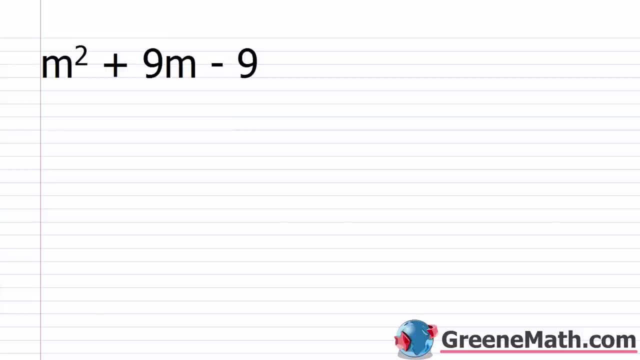 5 times 36 is plus 180. 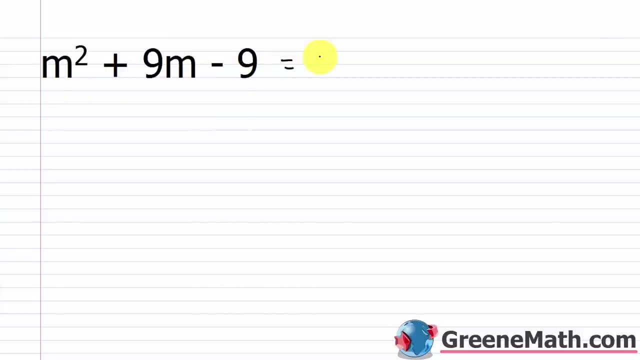 Let's take a look at m squared plus m here and m here. 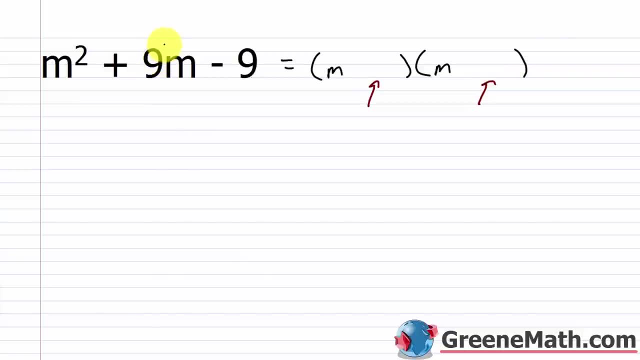 Now, for this spot and this spot, I need two integers whose sum is 9 and whose product is negative 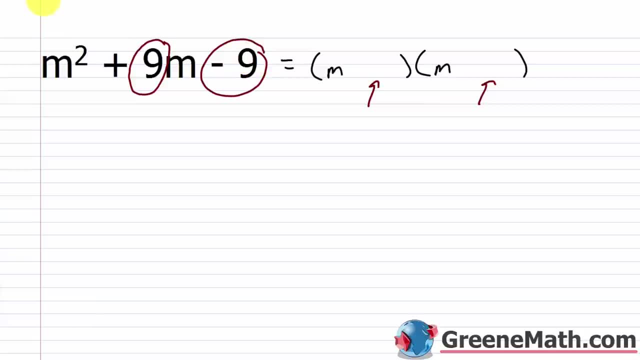 9. So let's think about the factors of just 9. 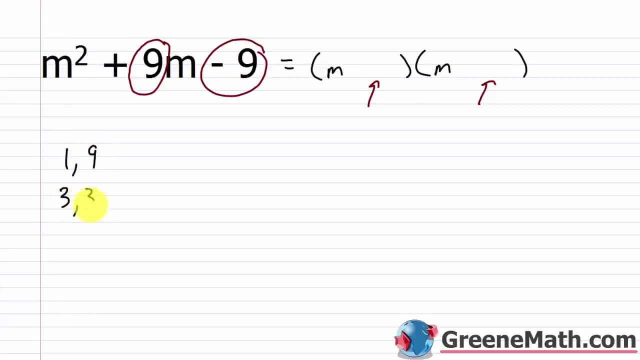 You have 1 and 9 and you have 3 and 3. That's it. I can't use 3 That's not ever going to work. 1 and 9, if I had 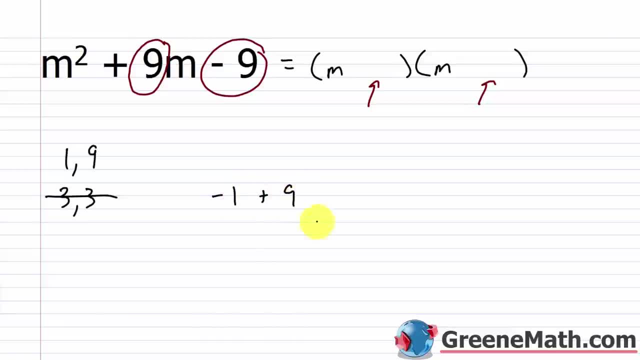 negative 1 plus positive nine that would give me positive eight and it would multiply to be negative nine but I don't 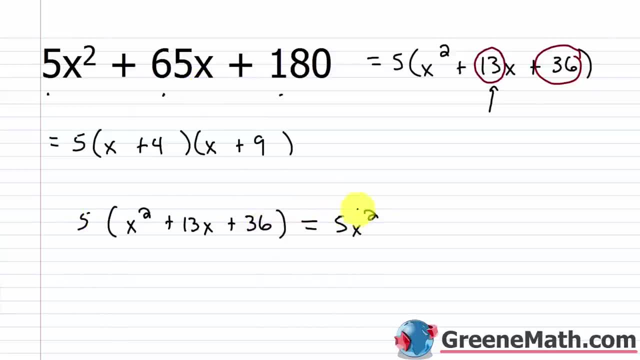 and you will get this back: 5 times x squared is 5x squared. 5 times 13x is plus 65x. 5 times 36 is plus 180. that's exactly what we started with, right there. alright, let's take a look at m squared plus 9x. 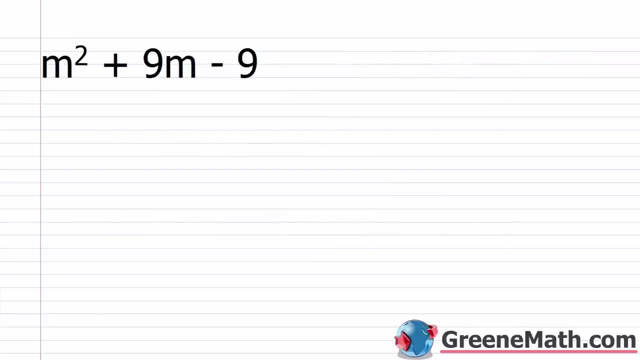 m minus 9, so this is one where we're going to have a problem. so again, you go ahead and start out. is there anything common to everything? no, there's not. m squared is the first term, so I know I have m here and m here. 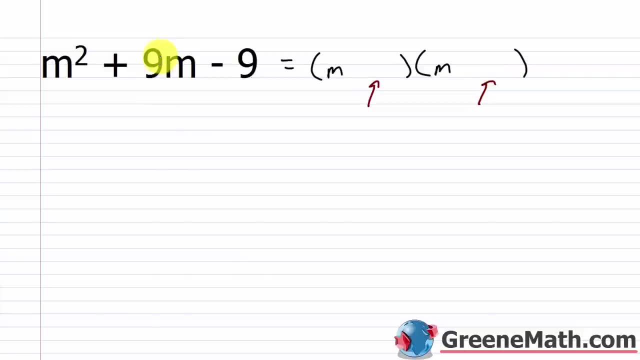 now for this spot and this spot. so I need two integers whose sum is 9 and whose product is negative 9. so let's think about the factors of just 9. you have 1 and 9, you have 3 and 3, that's it. 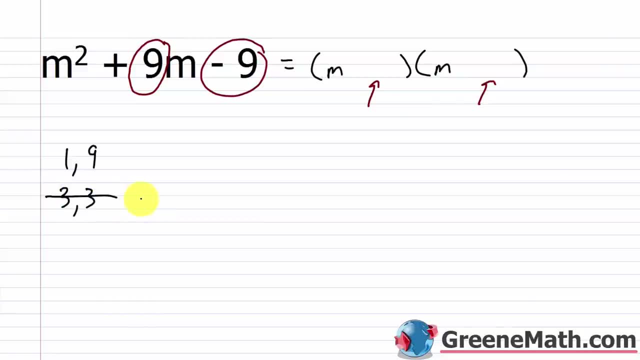 so I can't use 3 and 3. that's not ever going to work. 1 and 9: if I had negative 1 plus positive 9, that would give me positive 8 and it would multiply to be negative 9. but I don't want positive 8. 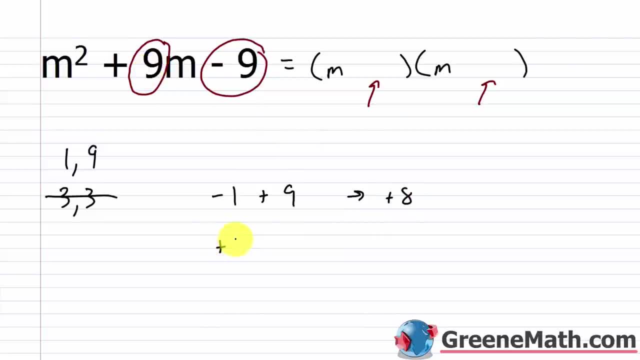 I want positive 9. if I used positive 1 and negative 9, well that's going to give me negative 8, and again I want positive 9. so there's not really anything else I can do. I have to use two different signs because the product here. 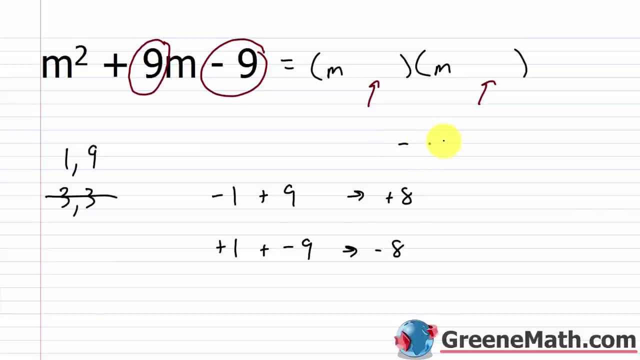 is a negative and a negative times. a positive yields a negative. I can't have two positives or two negatives involved, so I have to have one of these two work out. they don't, and so this polynomial is prime. alright, let's finish up with one. that's a little bit tricky. 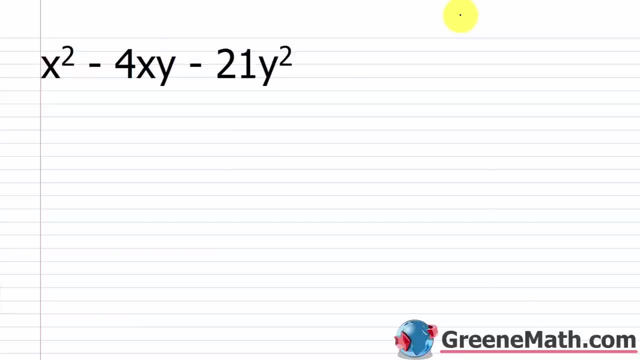 a lot of students see this and they get really, really confused. they're like: why is this? in this section, there are two variables involved, but what you're going to do is you're going to end up treating one of the variables as just a number. so let me kind of explain this to you. 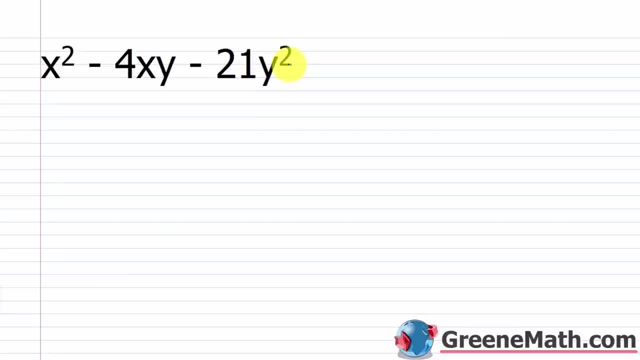 you have x squared minus 4xy minus 21y squared, the first variable that you see, the x squared. treat that like you normally would. so when you set this up, just go x here and x here. nothing else has changed. when you go to find these two positions, 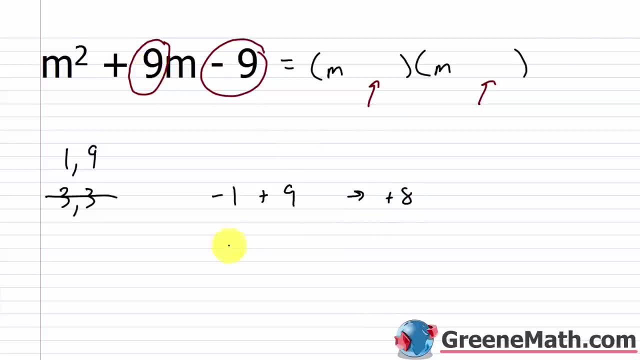 want positive eight I want positive nine if I used positive one and negative nine well that's 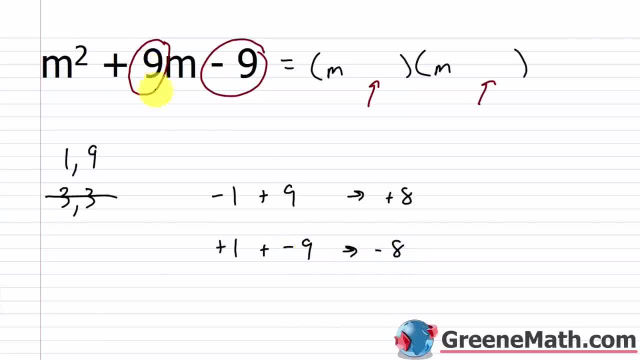 going to give me negative eight and again I want positive nine so there's not really anything else I can do I have to use two different signs because the product here is a negative and a negative 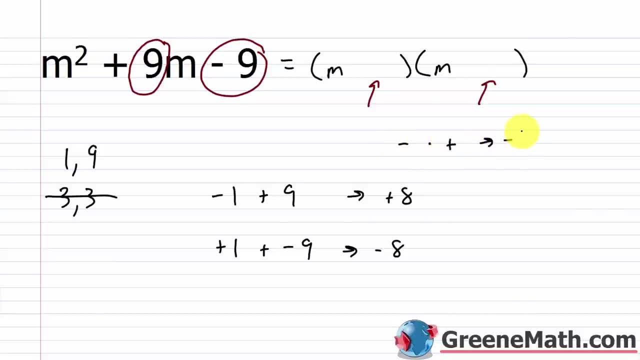 times a positive yields a negative I can't have two positives or two negatives involved so I have 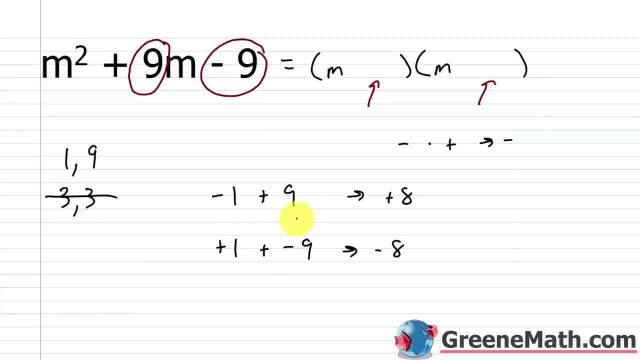 to have one of these two work out they don't and so this polynomial is prime all right let's finish up with one that's a little bit tricky a lot of students see this and they get really really confused they're like why is this in this section you have two variables involved but what you're going to do is you're going to end up treating one of the variables as just a number right so you're going to end up treating one of the variables as just a number right so you're going to end up treating one of the variables as just a number right so you're going to end up treating 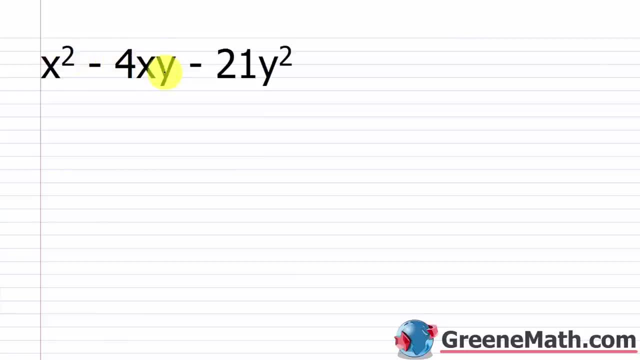 so let me kind of explain this to you you have x squared minus 4xy minus 21y squared the first variable that you see the x squared treat that like you normally would okay so when you set this up just go x here and x here nothing else has changed when you go to find these two positions here now what I'm looking for is I'm looking for a sum of not just negative four I'm looking for a negative four and I'm looking for a negative four and I'm looking for a negative four and I'm looking for a negative four y I'm looking for a sum of negative four y again the original variable the x squared don't include that but the other variable that's involved you will include that so in this case that's a y so you do negative four y then I want a product a product of this whole thing here negative 21y squared so just start out by thinking about the number 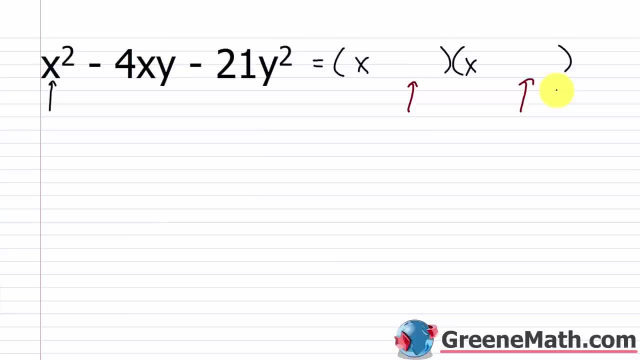 here now. what I'm looking for is: I'm looking for a sum of not just negative 4, I'm looking for negative 4y. I'm looking for a sum of negative 4y again. the original variable, the x squared, don't include that, but the other variable that's involved. 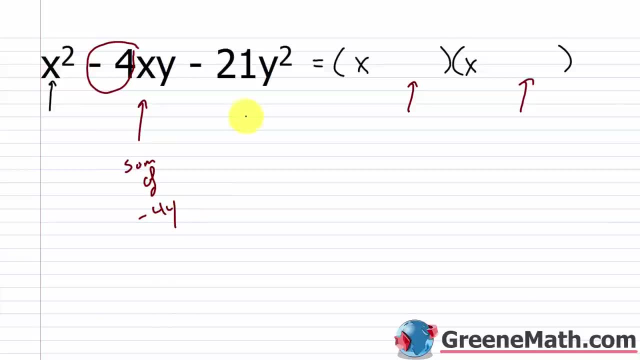 you will include that. so in this case that's a y, so you do negative 4y. then I want a product, this whole thing here negative 21y squared. so just start out by thinking about the number for 21. I have 1 and 21. 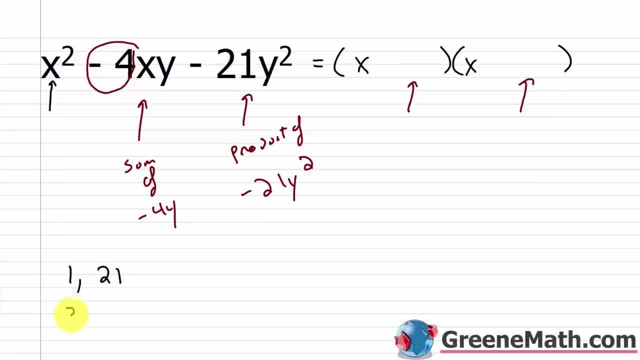 it's not divisible by 2, it is divisible by 3. I have 3 and I have 7. now I already know that if I work the signs correctly, I can get negative 4 out of 3 and 7. alright, I can do that. 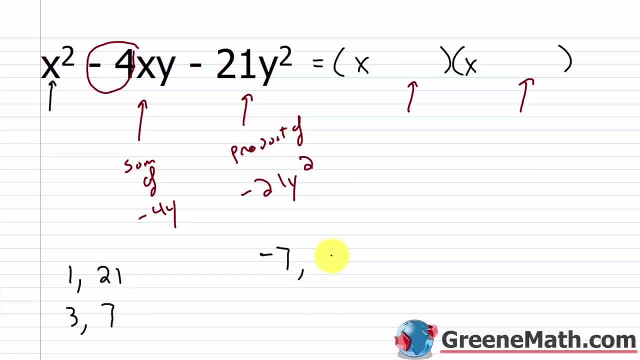 so let's think about that for a second. if I had a negative 7 plus 3, negative 7 plus 3 would give me negative 4. negative 7 times 3 would give me negative 21. so I could put negative 7 and plus 3. 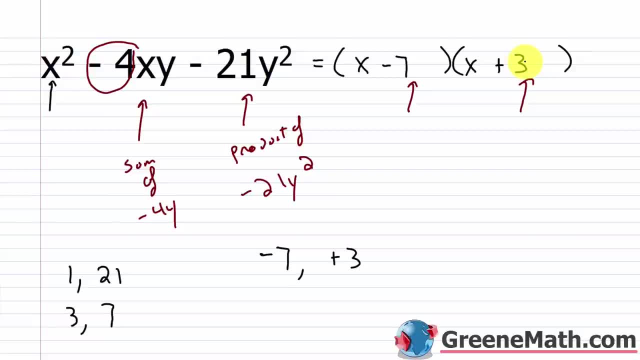 now what about the y part? well, you just throw it in there. just put a y here and a y here and think about it now. negative 7y times 3y would be negative 21y squared. negative 7y plus 3y would give you your negative 4y. 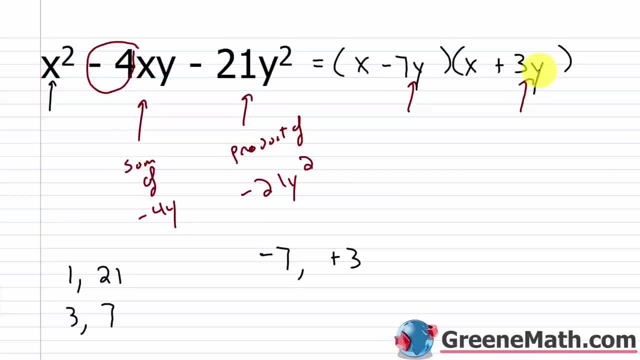 so everything works out there. when you see something like this, with two variables involved, it's no more difficult. you just have to kind of think about that second variable that you see as if it was a constant right, as if it was part of the number that you're working with. so, in other words, 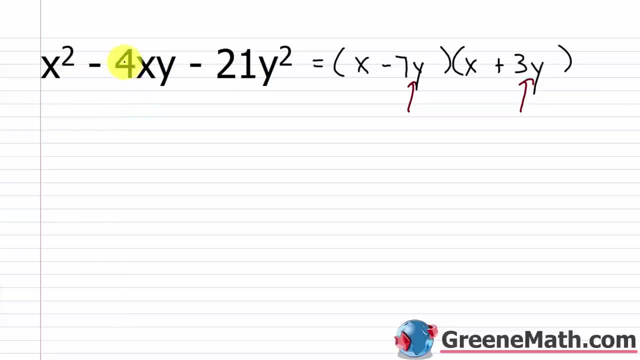 again, when you look for your sum, you take negative 4 and then you just include the y. so I'm looking for the sum of negative 4y and then, when you think about your product, include the whole thing. I'm looking for a product of negative 21y squared. 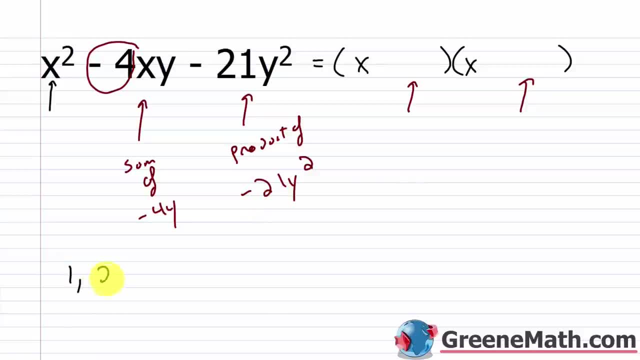 for 21 I have 1 and 21 it's not divisible by 2 it is divisible by 3 I have 3 and I have 7 now I already know that if I work the signs correctly I can get negative 4 out of 3 and 7 and I can do that so let's think about that for a second if I had a negative 7 and a positive 3 negative 7 plus 3 would give me negative 4 negative 7 times 3 would give me negative 21 so I could put negative 7 and plus 3 now what about the y part well you just throw it in there just put a y here and a y here and think about it now negative 7y times 3y would be negative 21y squared negative 7y plus 3y would give you your negative 4y so everything works out there when you see something like this with two variables involved it's no more difficult you just have to kind of think about that second variable that you see as if it was a constant right as if it was part of the number that you're working with so in other words again when you look for your sum you take negative 4 and then you just include the y so I'm looking for the sum of negative 4y and then when you think about your product include the whole thing I'm looking for a product of negative 21y squared so again I like to check things x times x is x squared outer x times 3y is plus 3xy inner negative 7y times x is minus 7xy these would combine together to be negative 4xy and then negative 7y times positive 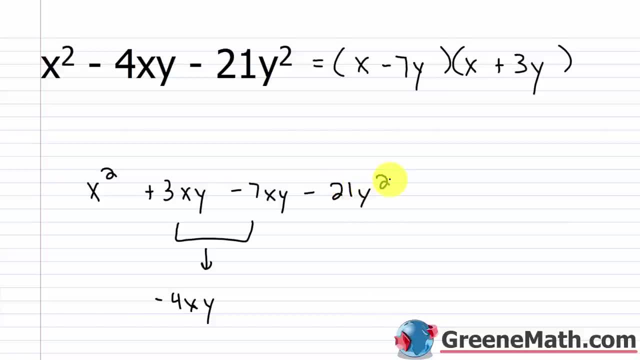 3y would be negative 21y squared so again if I combine like terms here I get x squared minus 4xy minus 21y squared which is exactly what I started with right there hello and welcome to algebra 1 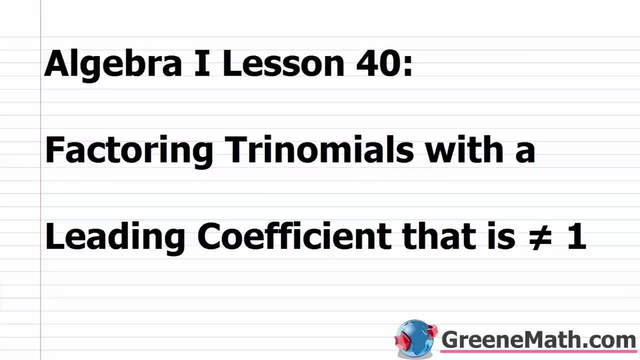 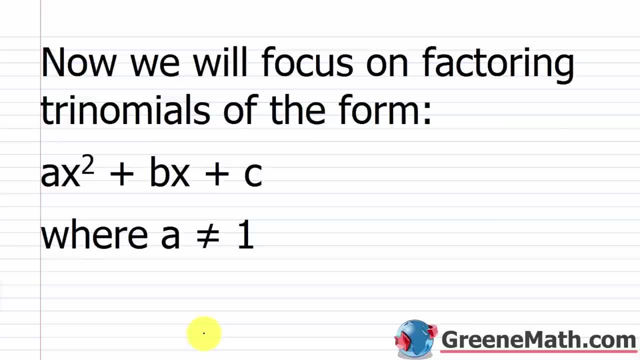 lesson 40. in this video we're going to learn about factoring trinomials with a leading coefficient that is not equal to 1 so in our last lesson we learned how to factor a trinomial that looks like this ax squared plus bx plus c or a the coefficient for the 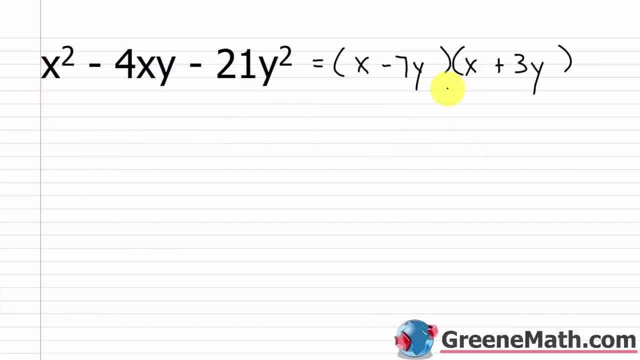 so again I like to check things. x times x is x squared outer. x times 3y is plus 3xy. inner negative 7y times x is minus 7xy. these would combine together to be negative 4xy and then negative 7y. 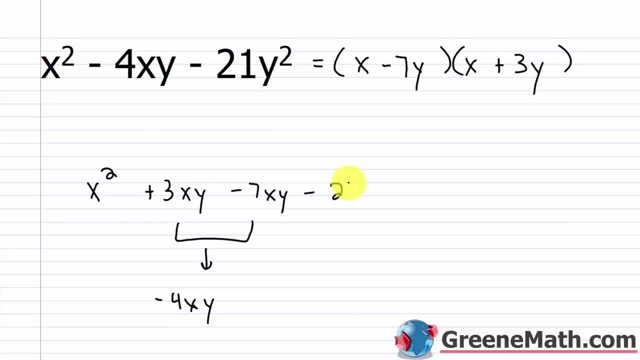 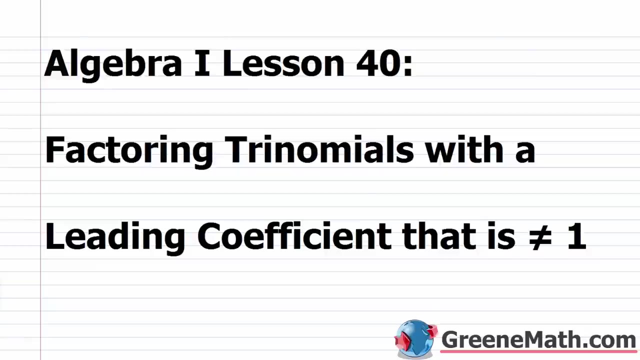 times positive, 3y would be negative 21y squared. so again, if I combine like terms here, I get x squared minus 4xy minus 21y squared, which is exactly what I saw when I started with right there. hello and welcome to algebra 1. 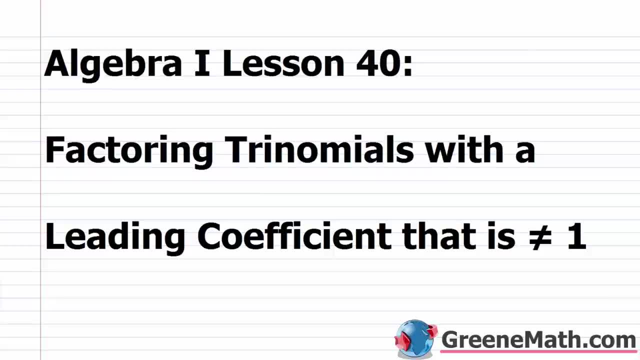 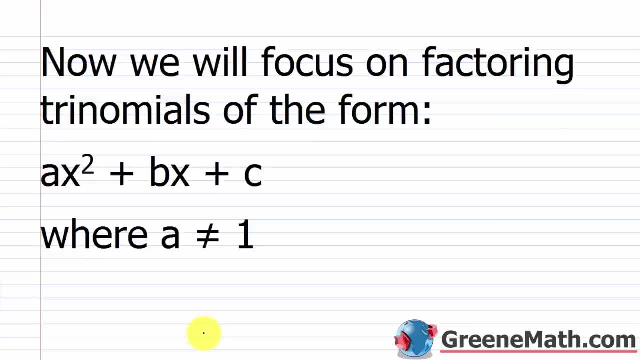 lesson 40 in this video we're going to learn about factoring trinomials with a leading coefficient that is not equal to 1. so in our last lesson we learned how to factor a trinomial that looks like this: ax squared plus bx. 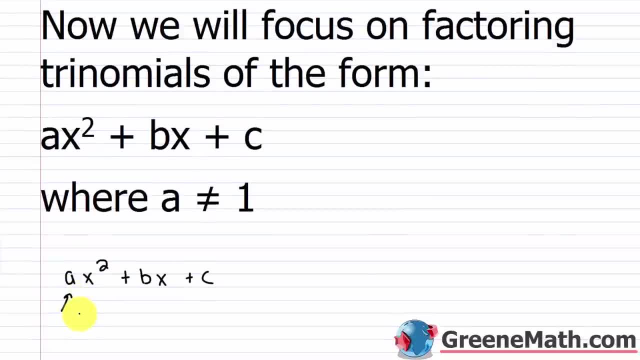 plus c or a, the coefficient for the x squared is a- 1. now this is the easiest scenario, like, let's say, x squared plus 5x plus 6. I would set this up as the product of two binomials. I know that, since the coefficient 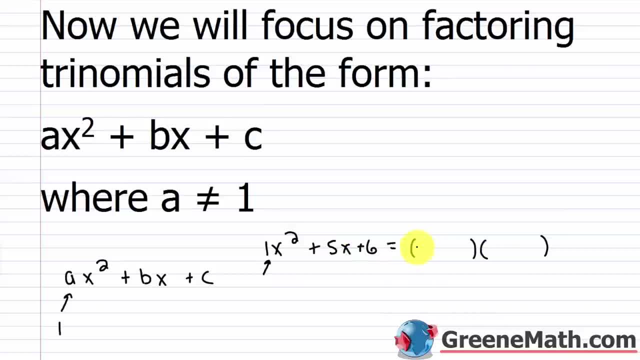 of this is 1. it's very easy to get the first two. so x goes here and x goes here, because x times x gives me that first term of x squared. then for these two missing parts here, I just need to figure out two integers whose sum is 5. 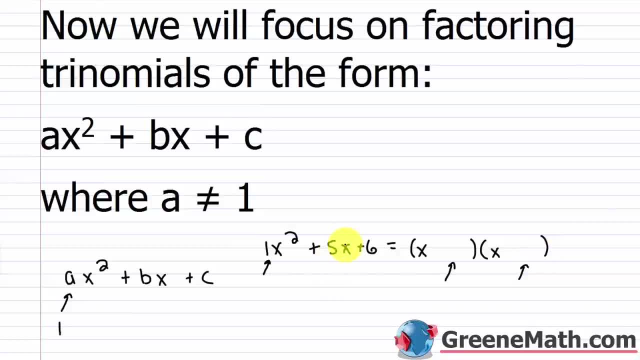 right, that middle term there the coefficient for the middle term, and whose product is that constant term 6. that's why we say a sum of b and a product of c. so this is b and this is c. alright, so once we figure that out, we just place those two integers. 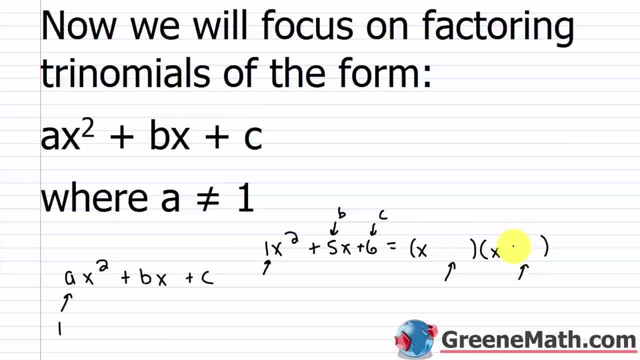 in those missing spots. so two integers that would multiply together to be 6, but sum to 5 would be positive 2 and positive 3. so x plus 2 times x plus 3. those two quantities multiplied together would give you x squared plus 5x plus 6. 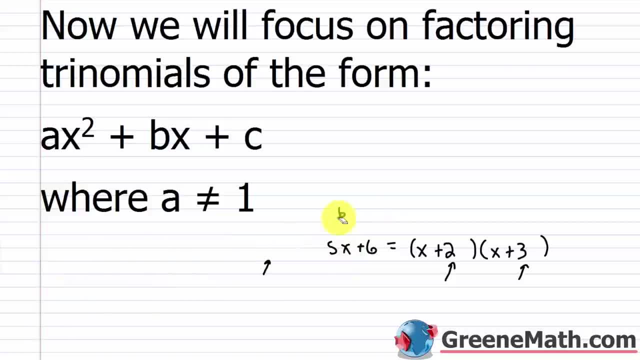 but this is the easy scenario to deal with. hopefully, at this point you've mastered that. we're now going to look at the harder part, which is to say, now we will focus on factoring trinomials of the form ax squared plus bx plus c. 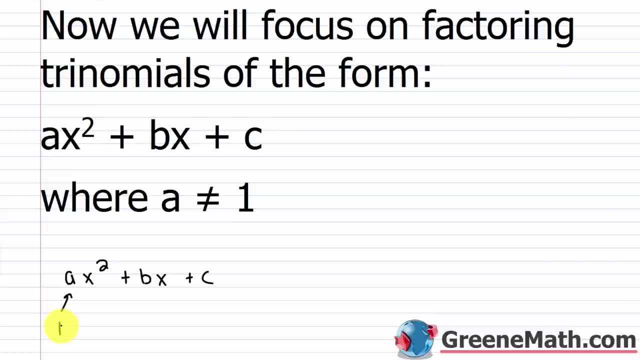 x squared is a 1 now this is the easiest scenario so if I had something like let's say x squared plus 5x plus 6 I would set this up as the product of two binomials I know that since the coefficient of this is 1 it's very easy to get the first two so x goes here and x goes here right because x times x gives me that first term of x squared then for these two missing parts here I just need to figure out two integers whose sum is 5 right that middle term there the coefficient for the middle term and whose product is that constant term 6 that's why 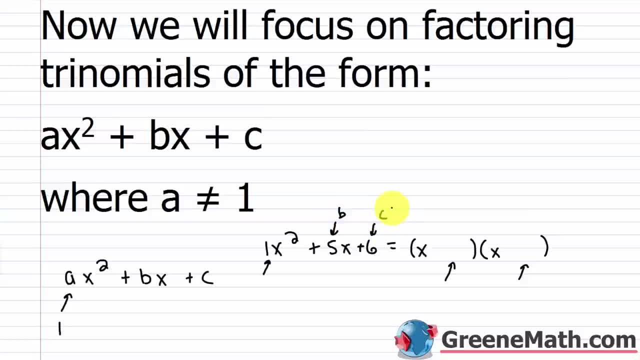 this is b and this is c all right so once we figure that out we just place those two integers in those missing spots so two integers that would multiply together to be 6 but sum to 5 would be positive 2 and positive 3 so x plus 2 times x plus 3 those two quantities multiplied together will give you x squared plus 5x plus 6 but this is the easy scenario to deal with hopefully at 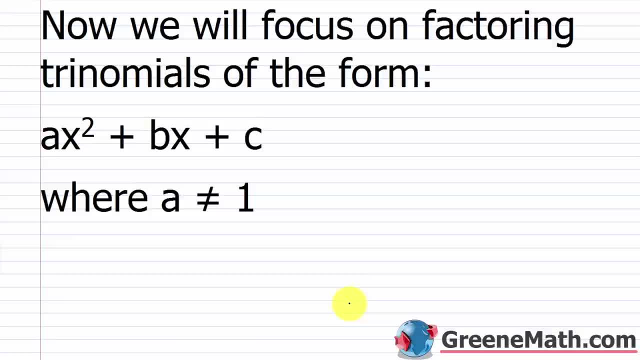 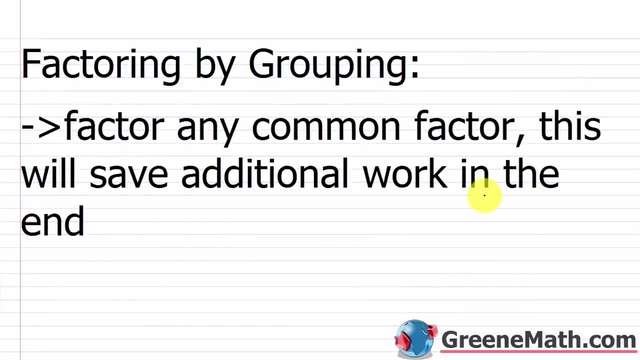 this point you've mastered that we're now going to look at the harder part which is to say now we will focus on factoring trinomials of the form ax squared plus bx plus c where a is not equal to 1 right so this will no longer be 1 so I can't just jump ahead and say okay this is x and this is x because you won't have that in each position anymore so that's going to be another unknown that you have to deal with so how do we do this so there's two main methods that pretty much everybody's textbook will rely on to show you how to do this so the first method is to factor a trinomial when the leading coefficient is not one now the first method relies on factoring by grouping this is the method I primarily use I still use it today I think this method is fast easy and efficient the other method is reverse foil I do not like this method personally I just I find it to be just a complete waste of my time it's trial and error and even though I'm pretty good at it it still ends up taking me longer in most cases so I'm going to teach you both because your teacher might require that you demonstrate the ability to do both so I want to cover everything completely but you get the same answer either way and this method is so much easier for me and I always use it I know there's some tricks out there on the internet you know whatever you find that works for you do it again I like this method it's never let me down 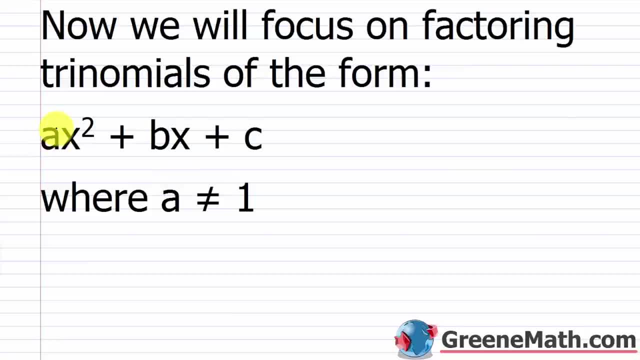 where a is not equal to 1, so this will no longer be 1, so I can't just jump ahead and say, ok, this is x, and this is x because you won't have that in each position anymore, so that's going to be another unknown. 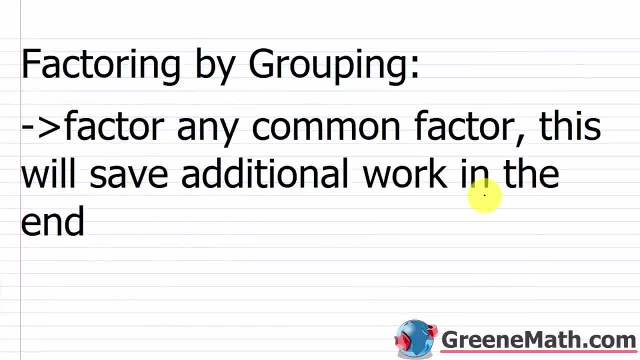 so how do we do this? so there's two main methods that pretty much everybody's textbook will rely on to show you how to factor a trinomial when the leading coefficient is not 1. now, the first method relies on factoring by grouping. this is the method I. 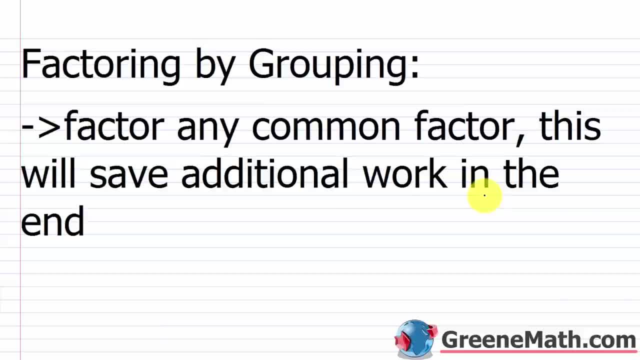 primarily use. I still use it today. I think this method is fast, easy and efficient. the other method is reverse foil. I do not like this method personally. I just find it to be just a complete waste of my time. it's trial and error and even though I'm pretty good at it- 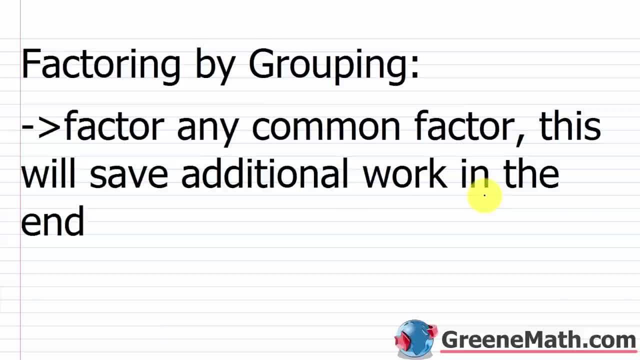 it still ends up taking me longer. in most cases, I'm going to teach you both, because your teacher might require that you demonstrate the ability to do both. so I want to cover everything completely, but you get the same answer either way, and this method is so much easier for me. 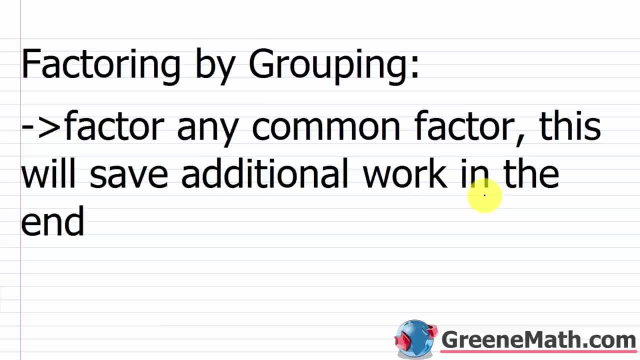 and I always use it, and I know there's some tricks out there on the internet, you know. whatever you find that works for you, do it again. I like this method. it's never let me down. so I'm going to start out with this. so the factoring by grouping method. 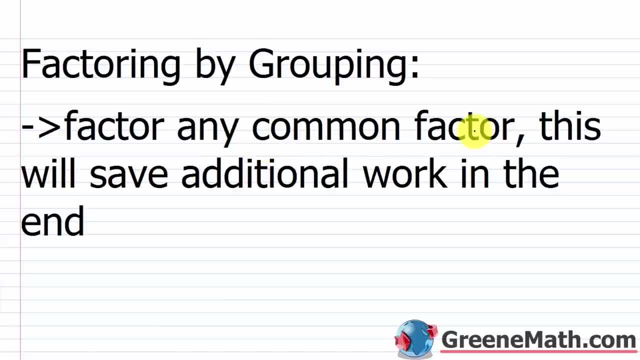 the first thing you're going to do. you do this always. you factor any common factor. this will save any additional work in the end. so if I have a trinomial and there's a factor that's common to everything that I can pull out, I'm going to go ahead and do that. 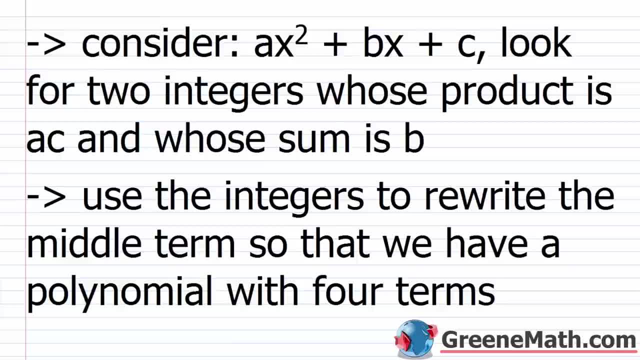 and then work with what's inside the parentheses. alright, so the next thing I want to do: consider the trinomial ax squared plus bx plus c. you want to look for two integers whose product is ac. before you were just looking for the product of c, but really, 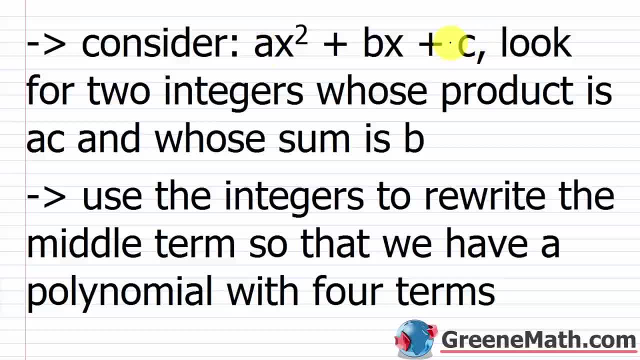 if a is one one times, c is just c, so it's the same thing. you're just adding this right here because now it's not equal to one, so the product is ac and the sum is b. so when you find those two integers, you're going to use the. 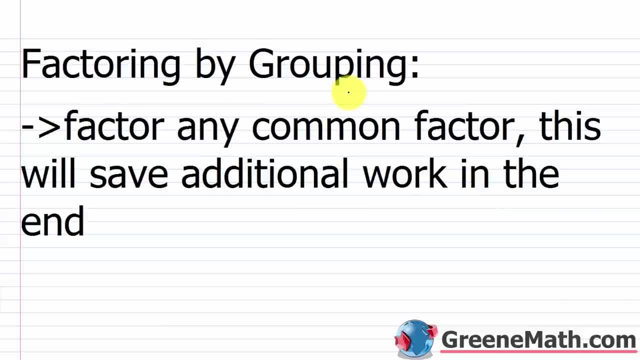 so I'm going to start out with this so the factoring by grouping method the first thing you're going to do you do this all the way you're going to do this all the way you're going to do 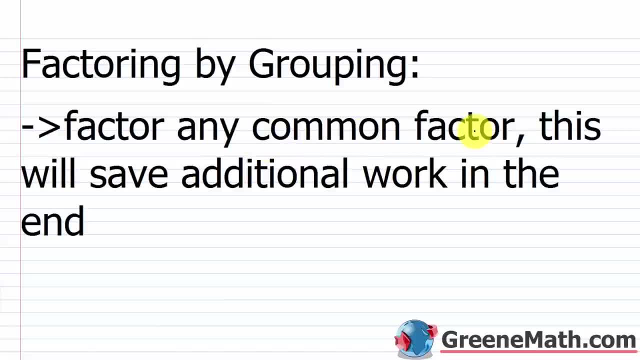 this all the way you factor any common factor this will save any additional work in the end so if I have a trinomial and there's a factor that's common to everything that I can pull out I'm going to go ahead and do that and then work with what's inside the parentheses all right 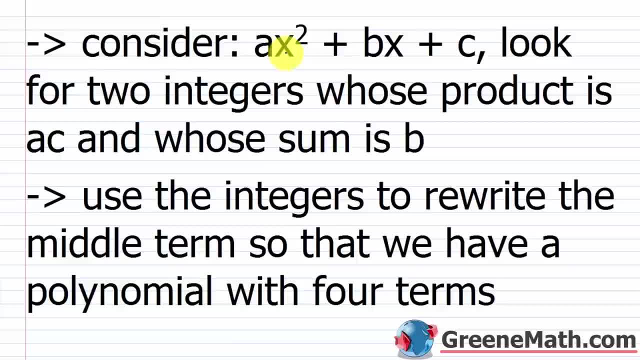 so the next thing I want to do consider the trinomial ax squared plus B X plus C you want to look for two integers whose product is a C before you were just looking for the product of 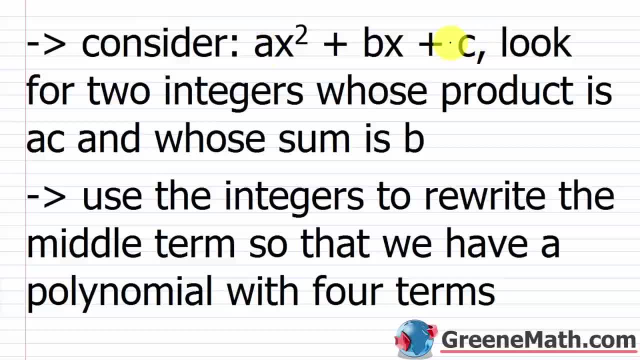 C but right now you're looking for the product of C so you're going to look for the product of C but right now you're looking for the product of C but right now you're looking for the product of C but really if a is 1 1 times C is just C so it's it's the same thing you're just adding this right here 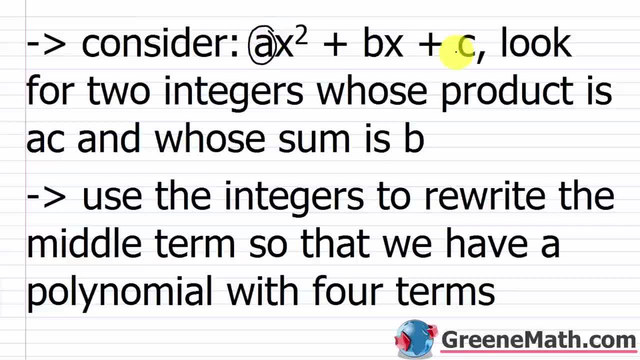 because now it's not equal to 1 so the product is a C and the sum is B so when you find those two integers you're going to use the integers to rewrite the middle term so that we have a polynomial with four terms and I know that might be a little confusing but once you see me do an example that's going to really resonate with you and show you how easy this is 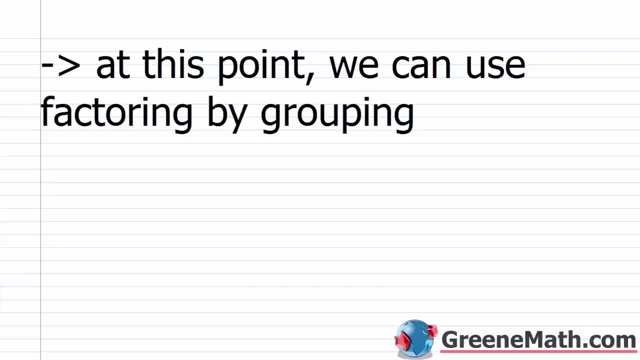 so then at this point we can use factoring by grouping all right so let's start out with the 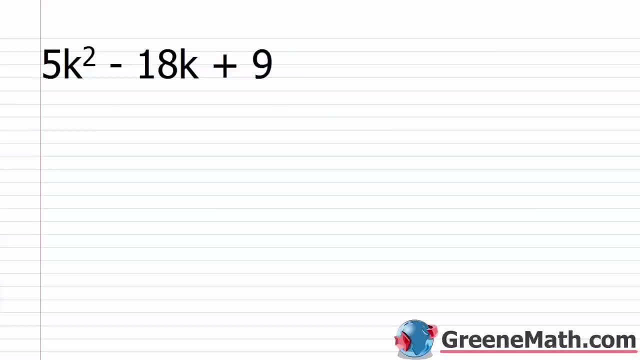 first example we have 5 K squared minus 18 K plus not so again this is my a this is my B and this is my C just for reference sake when I start I always look to see is there anything common to everything something I could pull up well there's not I have a 5 that's prime 18 is not divisible by 5 so I can just stop so nothing i could pull out so again i want two integers whose product is a times c and whose sum is b so b is negative 18 and ac five times nine is positive 45 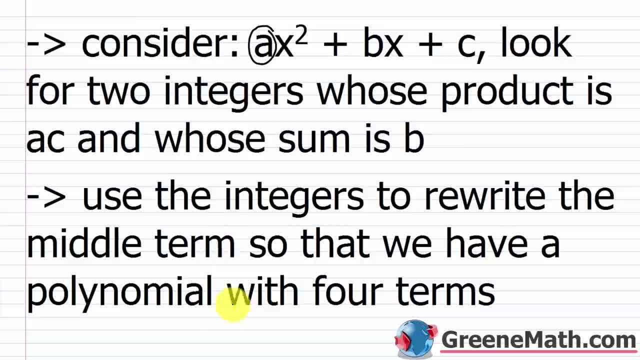 integers to rewrite the middle term so that we have a polynomial with four terms, and I know that might be a little confusing, but once you see me do an example that's going to really resonate with you and show you how easy this is. so then at this point we can use factoring. 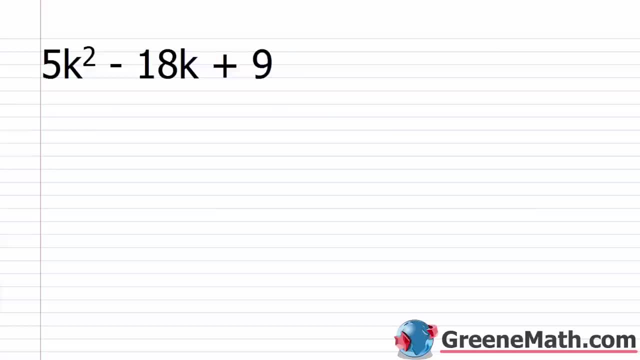 by grouping. alright, so let's start out with the first example. we have 5k squared minus 18k plus naught. so again, this is my a, this is my b and this is my c, just for reference sake. when I start I always look to see: is there anything? 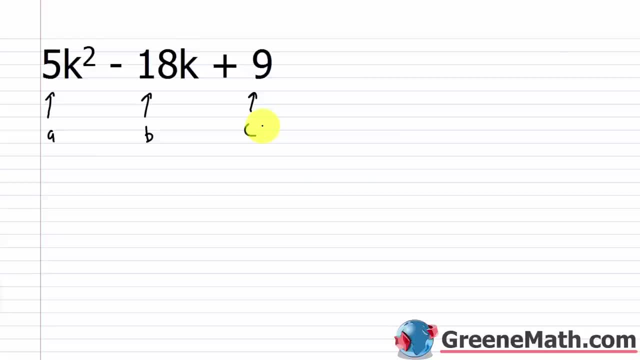 common to everything, something I could pull out? well, there's not. I have a 5 that's prime. 18 is not divisible by 5, so I could just stop. so nothing I could pull out. so again, I want two integers whose product is a times c. 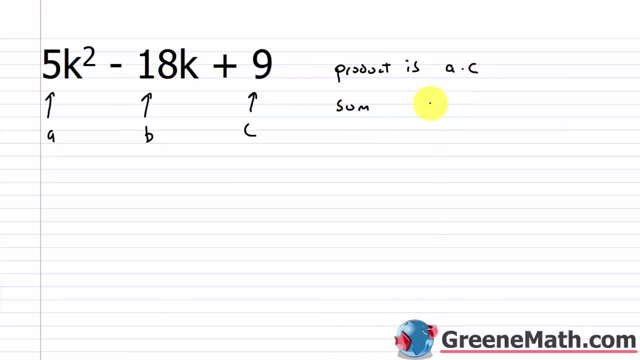 and whose sum is b. so b is negative 18 and ac 5 times 9 is positive 45. so we know we have to have two negative values right, because if I have a positive sum here and a negative sign here for the sum, I've got to have two negatives. 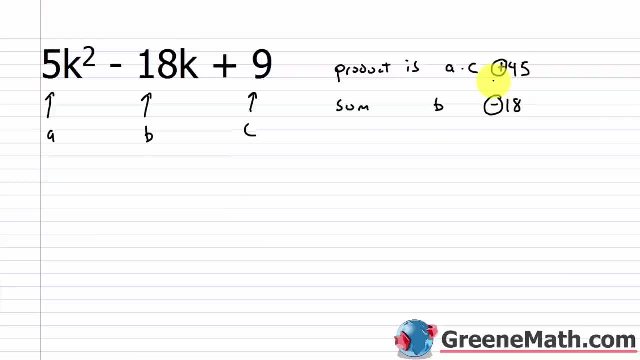 two negatives will multiply together to give me a positive. two negatives will sum together to give me a negative. so what are some factors of 45? and let's just think about positive factors and we'll make them negative. so we have 1 times 45, obviously that's. 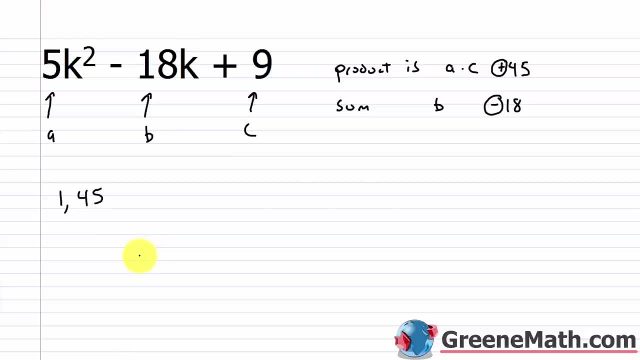 not going to work. not divisible by 2, it's not an even number. 4 plus 5 is 9, so it is divisible by 3, 45 divided by 3 is 15, so let's stop there. we could see that 3 plus 15 is 18. 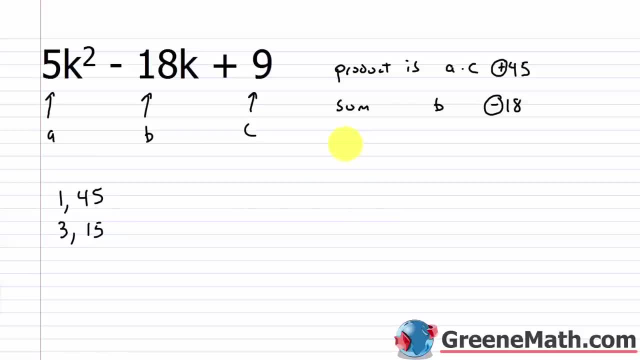 we just need to make the signs work and to do that we just make a negative 3 and a negative 15. now in the last kind of section, we were done at this point. we got our two integers, we threw them in and we were done. it's a little bit. 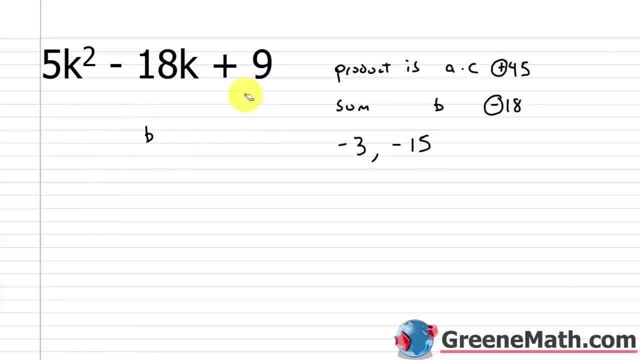 more work here. you've got to rewrite your middle term into a polynomial, that's four terms. so I'm going to take this and write it as 5k squared minus 15k, minus 3k plus 9, and I did two things there that I want to. 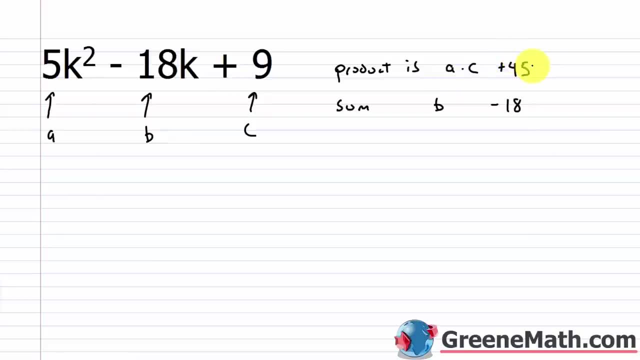 so we know we have to have two negative values right because if i have a positive sign here and a negative sign here for the sum i've got to have two negatives two negatives will multiply together give me a positive two negatives will sum together to give me a negative so what are some factors of 45 and let's just think about positive factors and we'll make them negative so we have 1 times 45 obviously that's not going to work not divisible by 2 it's not an even number 4 plus 5 is 9 so it is divisible by 3 45 divided by 3 is 15 so let's stop there we can see that 3 plus 15 is 18 we just need to make the signs work and to do that we just make a negative 3 and a negative 15 now in the last kind of section we were done at this point we got our two integers we threw them in and we were done it's a little bit more work here you've got to rewrite your 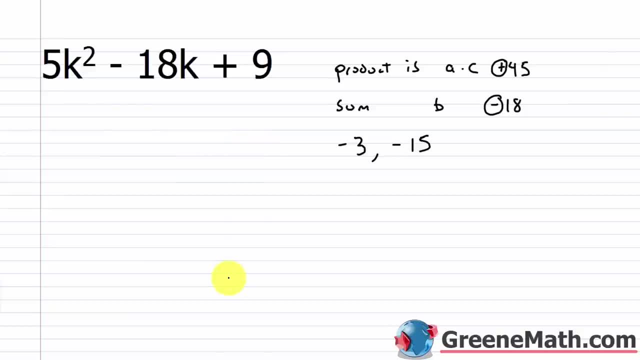 middle term into a polynomial that's four terms so i'm going to take this and write it as 5k squared minus 15k minus 3k plus 9 and i did two things there that i want to explain the first thing is 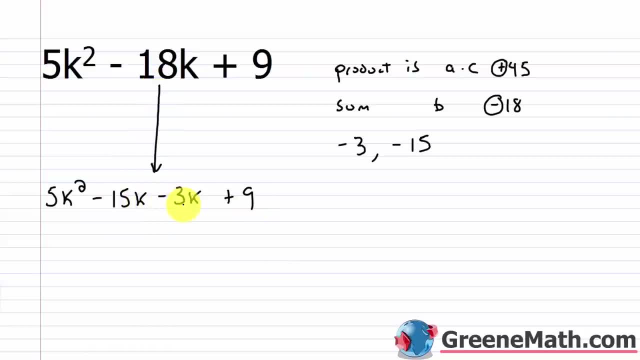 i'm going to write the middle term as negative 15k minus 3k i have not changed the value of this polynomial negative 15k minus 3k if i combine like terms i'm going to get negative 18k that's perfectly legal we've seen that with fractions and all kinds of other stuff where we change what 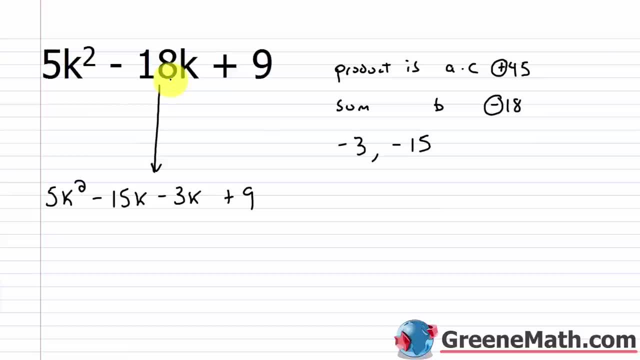 it looks like but the value is the same now the second thing is i put 15 next to 5 because i know 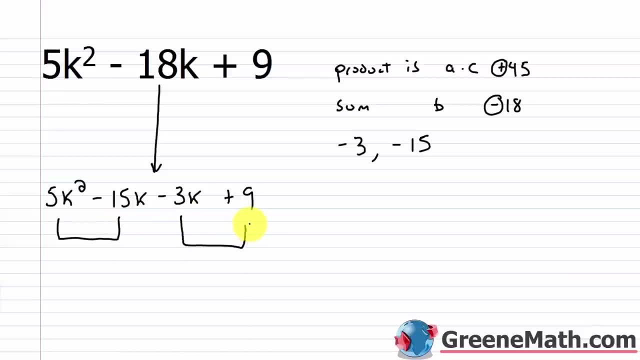 they have a common factor of 5 i put 3 next to 9 because i know they have a common factor of 3 so i did that because remember if you're factoring by grouping you want to put your groups together in a way to where you know you have some common factor you can pull out so that's why i did that 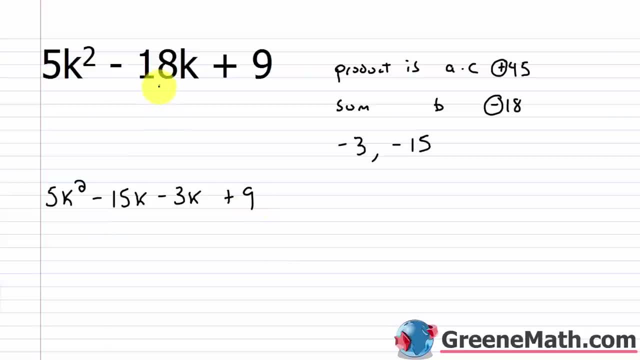 explain. the first thing is that I rewrote the middle term as negative 15k minus 3k. I have not changed the value of this polynomial: negative 15k minus 3k. if I combine like terms, I'm going to get negative 18k. that's perfectly legal. 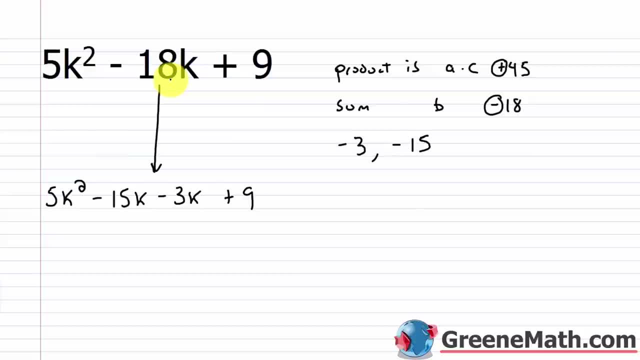 we've seen that with fractions and all kinds of other stuff, where we change what it looks like, but the value is the same. now the second thing is I put 15 next to 5, because I know they have a common factor of 5. I put 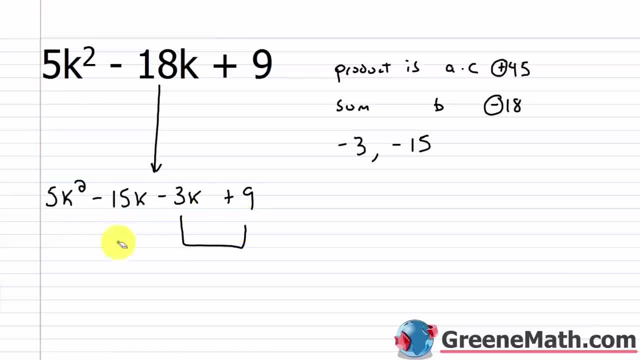 3 next to 9, because I know they have a common factor of 3. so I did that because, remember, if you're factoring by grouping, you want to put your groups together in a way to where you know you have some common factor you can pull out. so that's why I did that. 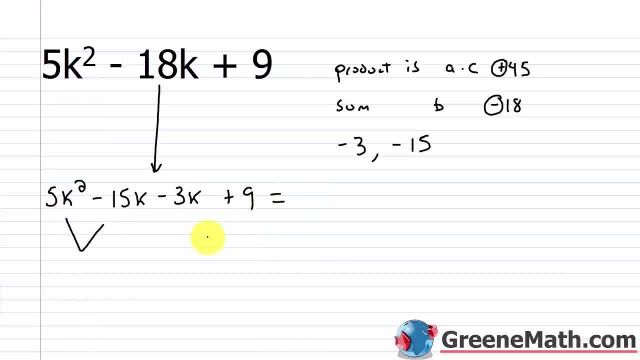 alright. so now we're going to factor by grouping, so in the first group I can pull out a 5k, so I would have 5k. outside, inside I would have a k minus a 3, and then in the second group I would pull out. 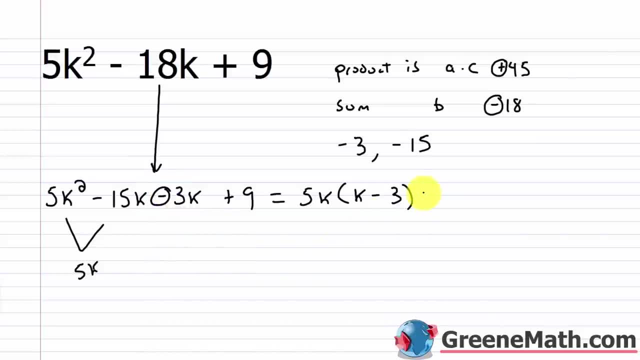 a negative 3. so I'm going to put plus negative 3 times what's left in there you would have a positive k minus 3. so you can see you have a common binomial factor of k minus 3, common binomial factor. so let's factor that guy out. 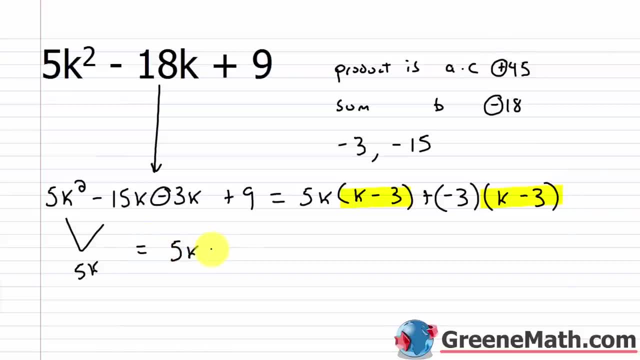 so this is equal to 5k minus 3 times k minus 3. if I took out the k minus 3 and put that here, what would be left is a 5k minus 3, so that's why I have 5k minus 3. 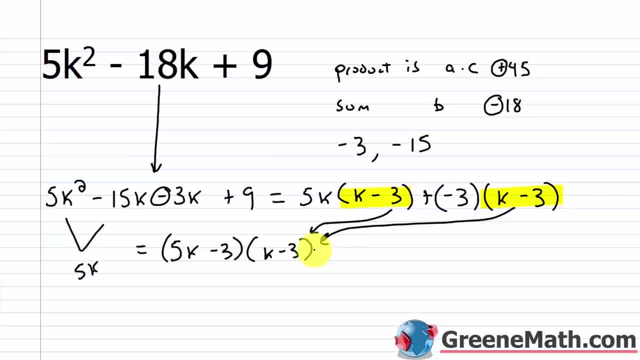 times k minus 3 and I'm done. I've completely factored this guy as long as I didn't have a common factor when I started. I won't have one in here that requires additional work. I should be done. the only thing I have to do now is check 5k times k. 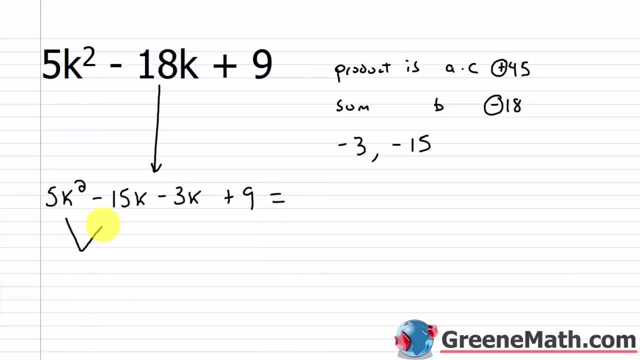 all right so now we're going to factor by grouping so in the first group i can pull out a 5k so i would have 5k outside inside i would have a k minus a 3 and then in the second group i would pull out a negative 3 so i'm going to put plus negative 3 times what's left in there you would have a positive k minus 3 so you can see you have a common binomial factor of k minus 3 common binomial factor so let's factor that guy out so this is equal to 5k minus 3 times k minus 3 if i took out the k minus 3 and put that here what would be left is a 5k minus 3. And I'm done. I've completely factored this guy. 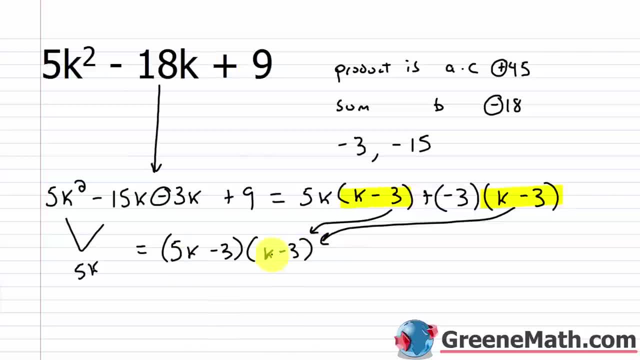 As long as I didn't have a common factor when I started, I won't have one in here that requires additional work. I should be done. The only thing I have to do now is check. 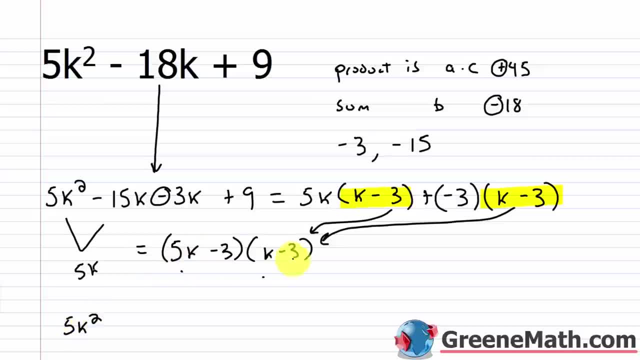 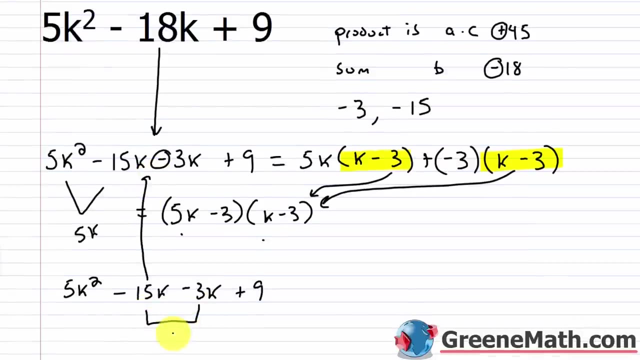 5k times k is 5k squared. 5k times negative 3 is minus 15k. Negative 3 times k is minus 3k. And then negative 3 times negative 3 is plus 9. So you can see I got exactly back what I had here. If I combine like terms, I'd get negative 18k in the middle. And then I would have exactly what I started with there. 5k squared minus 18k plus 9. Okay, let's take a look at another one. 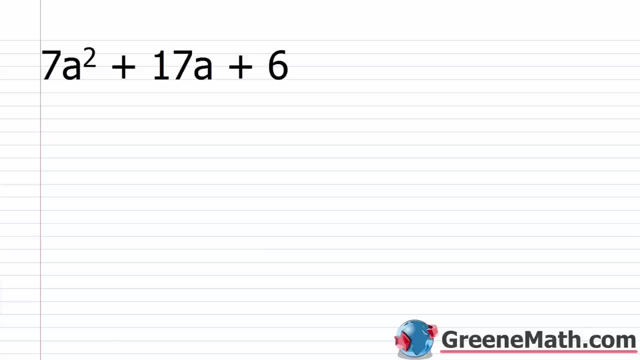 So we have 7a squared plus 17a plus 6. So again, I'm looking for two integers whose product is ac. So again, I'm looking for two integers whose product is ac. 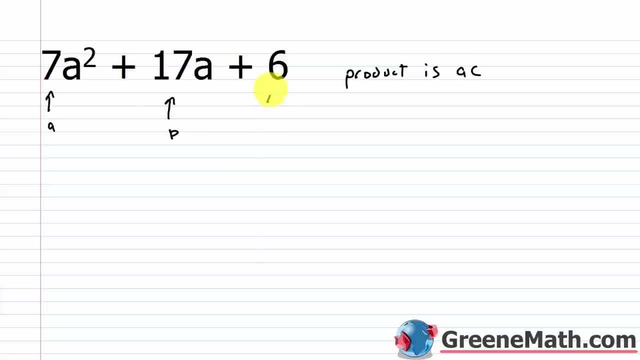 So again, this is a, this is b, and this is c. And I know this is ultra confusing because I now have a variable that's a. Okay, I have a variable that's a. But you can kind of ignore that. Typically, we have what? We have ax squared plus bx plus c. 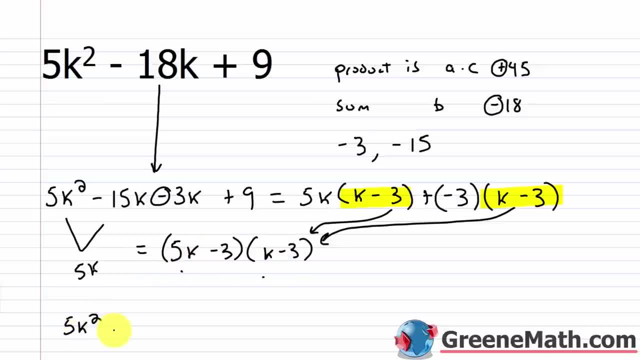 is 5k. squared 5k times negative 3 is minus 15k. negative 3 times k is minus 3k, and then negative 3 times negative, 3 is plus naught. so you can see I got exactly back what I had here if I combine. 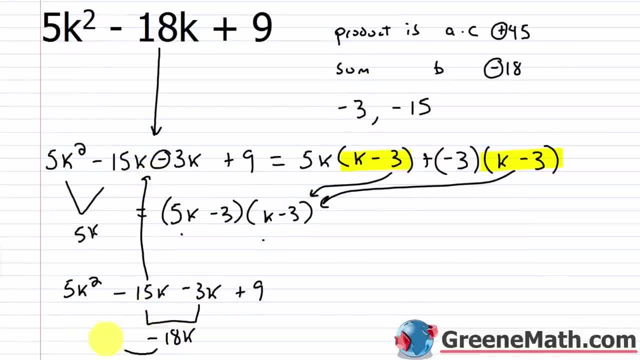 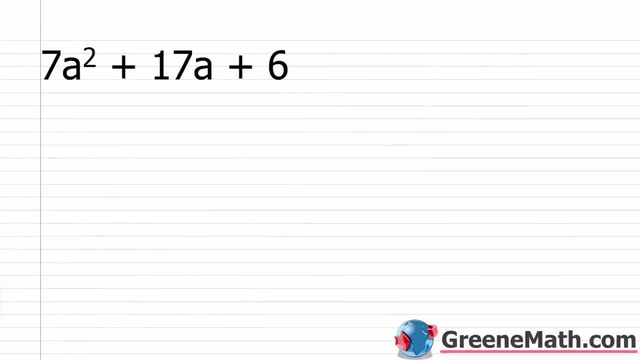 like terms. I'd get negative 18k in the middle, and then I would have exactly what I started with there: 5k squared minus 18k plus naught. okay, let's take a look at another one. so we have 7a squared plus 17a. 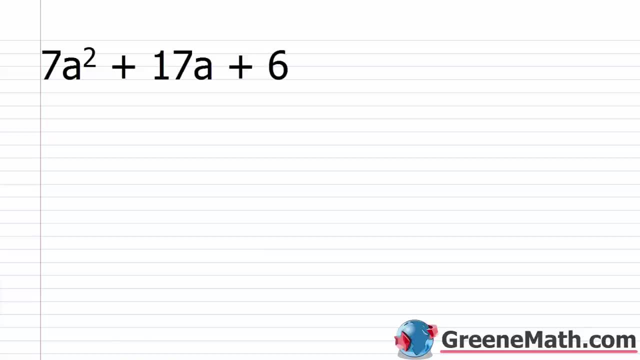 plus 6. so again I'm looking for two integers whose product whose product is ac. so again, this is a, this is b and this is c, and I know this is ultra confusing because I now have a variable that's a, I have a variable that's a, but you can kind of 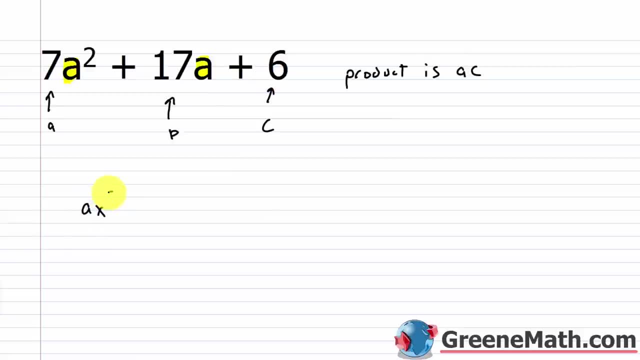 ignore that. typically we have what we have: ax squared plus bx plus c. so the coefficient for the square term- in this case it happens to be an, a. it's a squared is denoted with a when we talk about a generic formula. so it's just whatever the coefficient on the square term is. 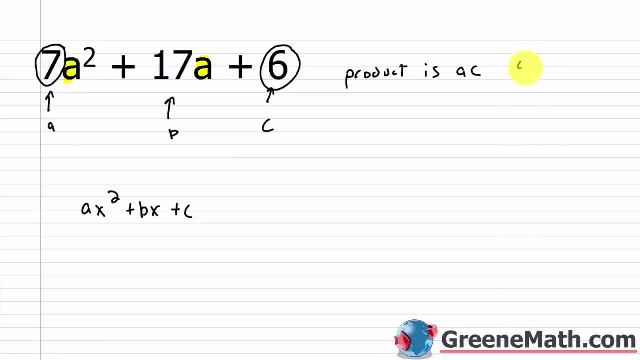 times whatever that constant is. so 7 times 6 is 42, and then sum is b, which is 17, right? so whatever that number is okay, including the sign for your middle term, right? in this case, that's 17, alright. so moving on, what two numbers would 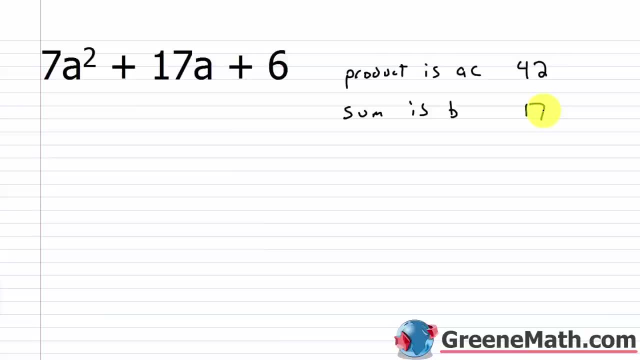 multiply together to give me 42 and sum to 17. well, we think about the factors of 42. we've got 1 and 42, we've got 2 and 24. then 4 plus 2 is 6, 6 is divisible by 3. so 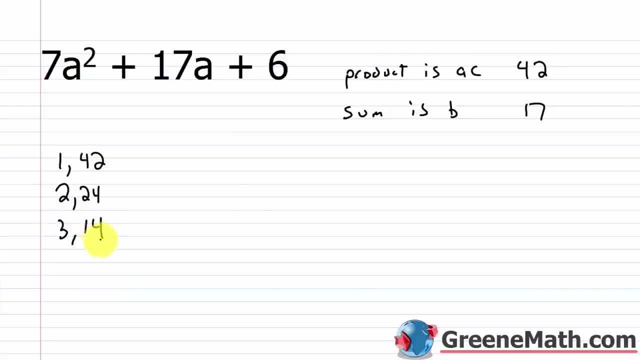 42 is 42 is 3 times 14 and that looks like that would work right. 3 plus 14 is 17, 3 times 14 is 42. so again, at this point we're not done. right before we were done, we found our two integers. we throw them in. 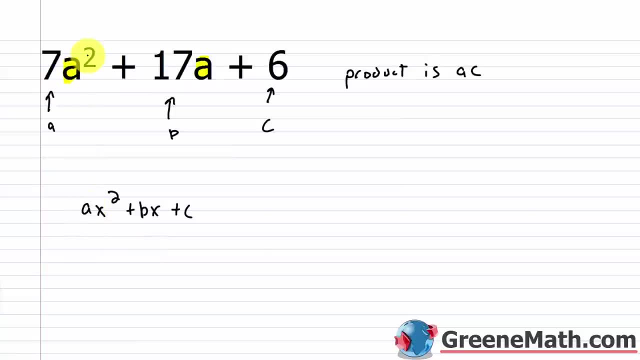 So the coefficient for the square term, in this case it happens to be an a, it's a squared, is denoted with a when we talk about a generic formula. 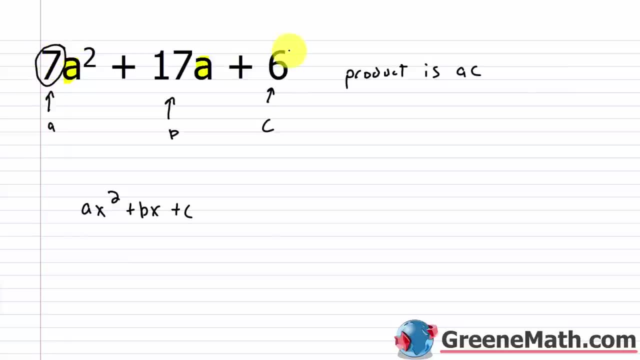 So it's just whatever the coefficient on the square term is times whatever that constant is. 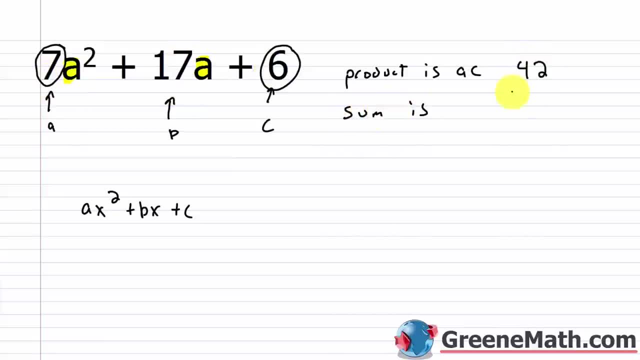 And then sum is b, which is 17. Right? 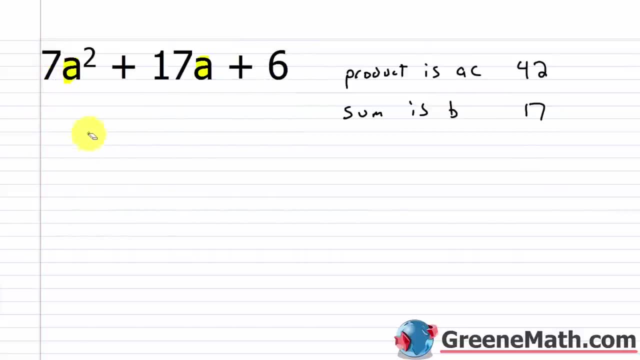 So whatever that number is, okay, including the sign for your middle term. In this case, that's 17. 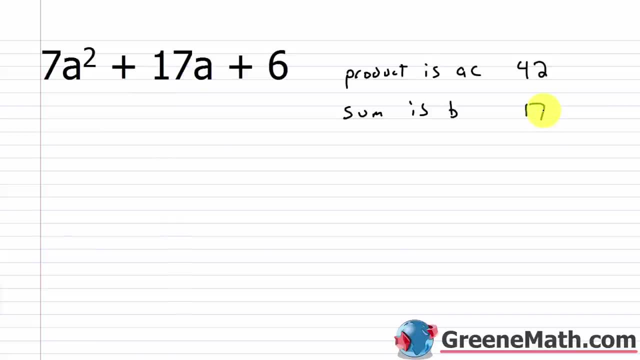 All right, so moving on. What two numbers would multiply together to give me 42 and sum to 17? 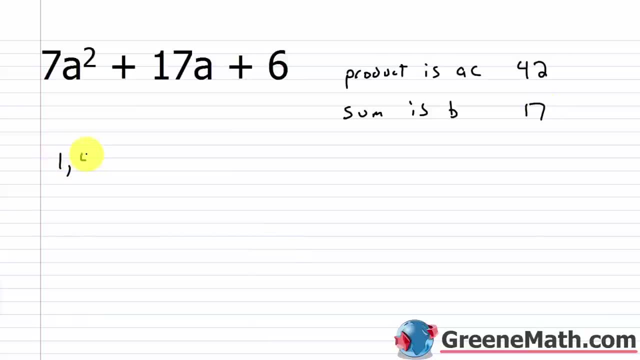 Well, we think about the factors of 42. We've got 1 and 42. We've got 2 and 24. Then 4 plus 2 is 6. 6 is divisible by 3, so 42 is. 42 is 3 times 14. And that looks like that would work, right? 3 plus 14 is 17. 3 times 14 is 42. 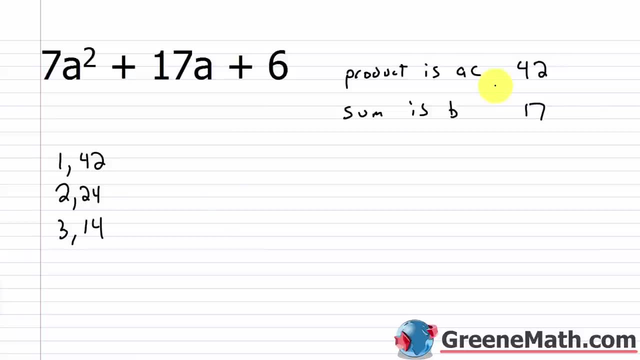 So again, at this point, we're not done, right? Before we were done, we found our two integers. We throw them in. We're not done. 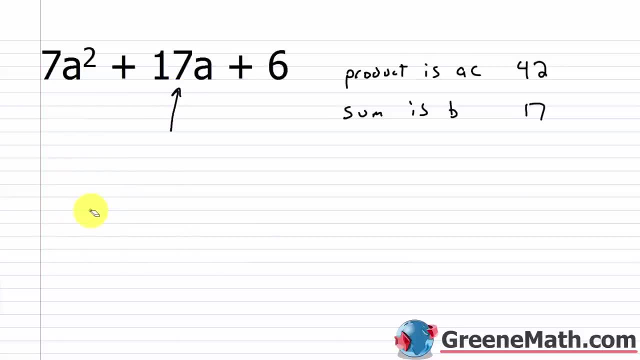 We're going to use that to rewrite that middle term. So we're going to break it up into 7a squared plus 14a plus. 3a plus 6. And again, notice that I put 7 next to 14, 3 next to 6, right? Because I know I can pull a 7 out of here and a 3 out of here. So that's why I did that. 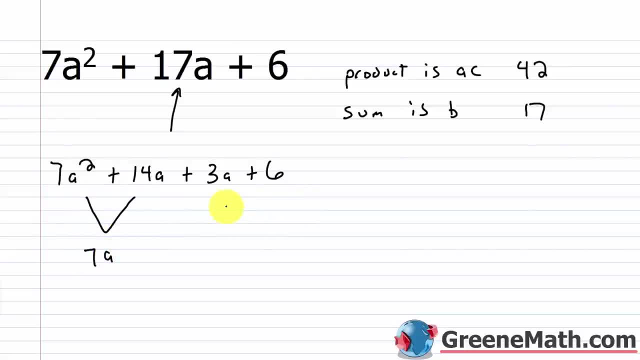 All right, so the GCF for these two would be 7a. The GCF for these two would be 3. So then equals, if I pull a 7a out of there, I'll have 7a times a plus 2. 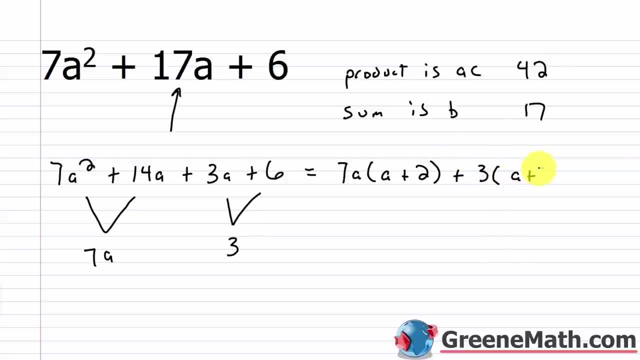 If I pull a 3 out of here, I'll have 3 times a plus 2. So if I factor out that. Common binomial factor of a plus 2. 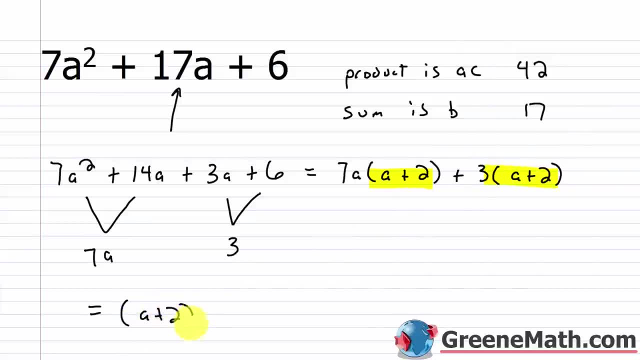 If I pull that guy out, I'll have a plus 2. And what's left? I'll have a 7a plus a 3. 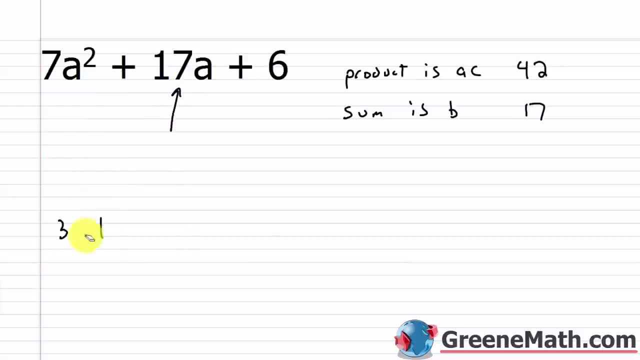 we're not done. we're going to use that to rewrite that middle term. so we're going to break it up into 7, a squared plus 14, a plus 3, a plus 6, and again notice that I put 7 next to 14. 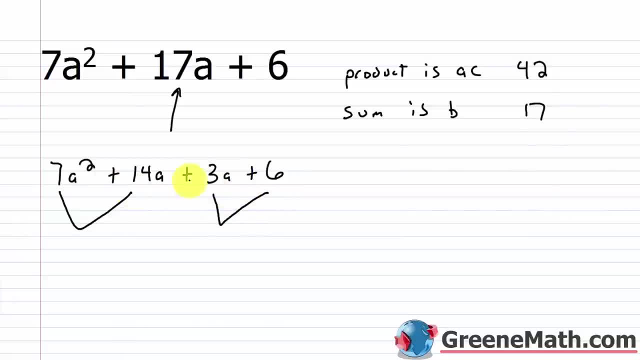 3 next to 6, right, because I know I can pull a 7 out of here and a 3 out of here, so that's why I did that. alright, so the GCF for these two would be 7. a the GCF for these two would be 3. 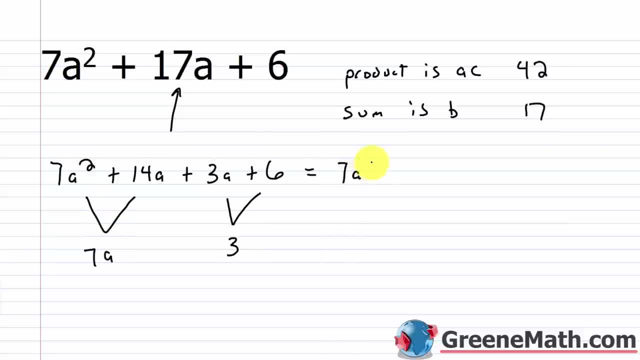 so then equals: if I pull a 7 a out of there, I'll have 7 a times a plus 2. if I pull a 3 out of here, I'll have 3 times a plus 2. so if I factor out that common binomial factor, 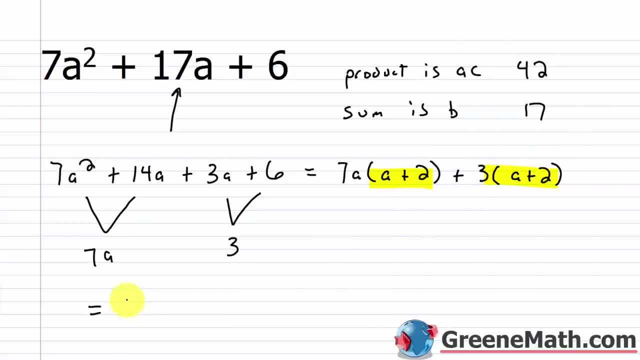 of a plus 2. if I pull that guy out, I'll have a plus 2, and what's left? I'll have a 7 a plus a 3. so a plus 2 times 7 a plus 3- and again- check this with FOIL- a times 7 a is. 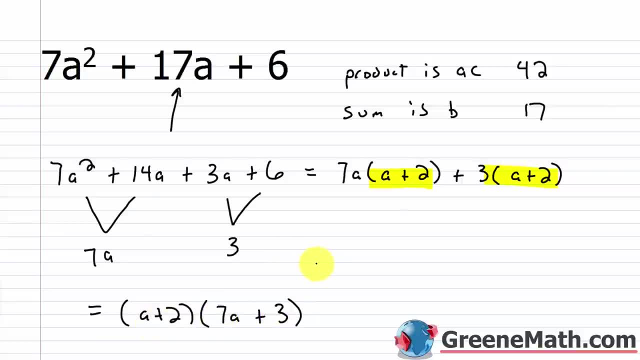 7 a squared a times 3 is 3 a, 2 times 7 a is plus 14 a. so 14 a plus 3 a would be 17 a, and then 2 times 3 is 6, so you get 7 a. 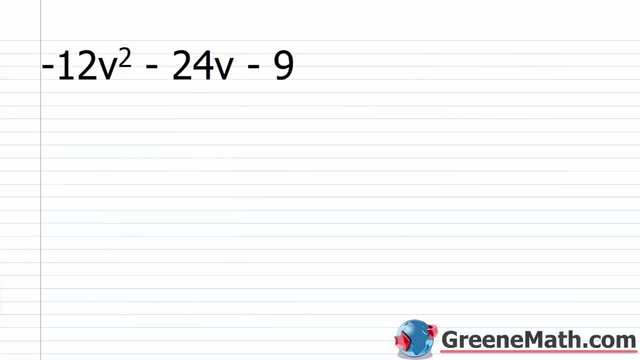 squared plus 17. a plus 6. alright, let's try. negative 12 v squared minus 24. v minus 9. so everything is negative here. so I know I can pull that out to start and make my life a lot easier. I hate working with negatives. everybody does, I also. 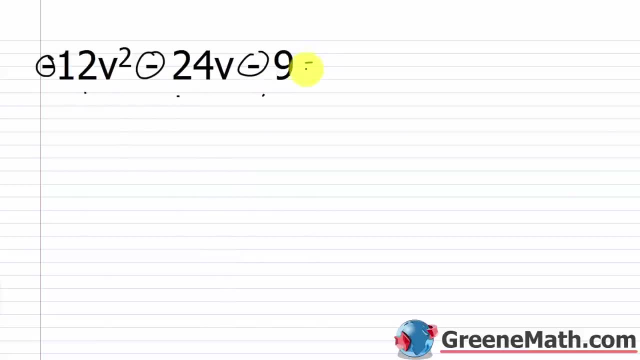 notice that everything is divisible by 3. so let's pull out a negative 3 and we'd have 4 v squared plus 8 v plus 3. so now I just need to worry about what the inside of the parentheses here would factor to. so again I'm looking at. 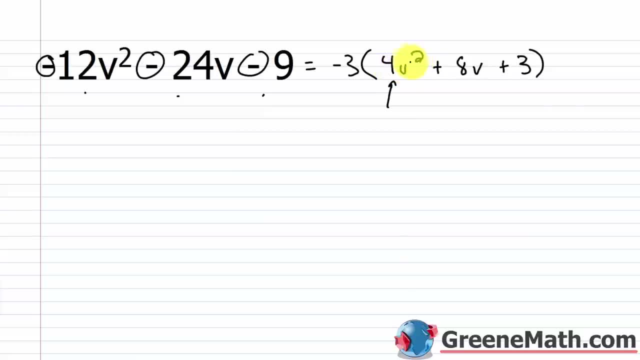 the a, or the coefficient for the squared term, and I'm looking for the c, which is the constant. so multiply those two together: 4 times 3 is 12, so product of 12. and then I'm looking for a sum of 8, so what? 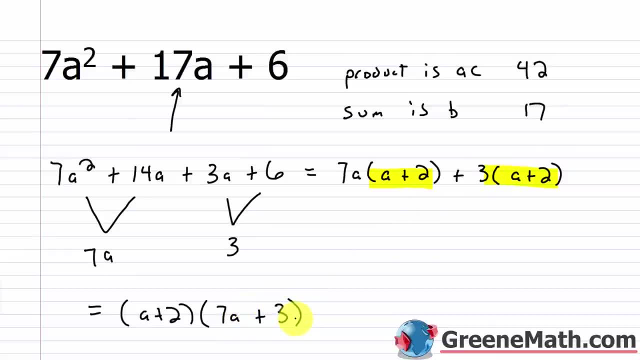 So a plus 2 times 7a plus 3. And again, check this with FOIL. a times 7a is 7a squared. a times 3 is 3a. 2 times 7a is plus 14a. So 14a plus 3a would be 17a. And then 2 times 3 is 6. So you get 7a squared. Plus 17a plus 6. 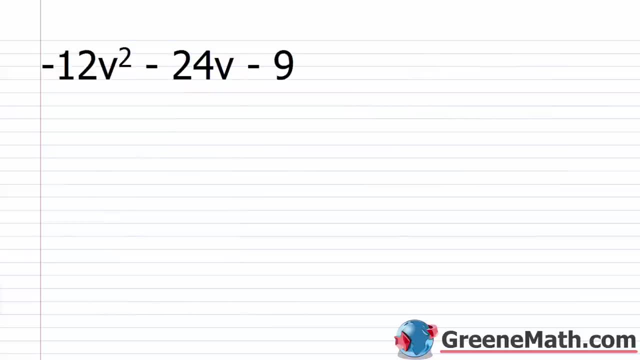 All right, let's try negative 12v squared minus 24v minus 9. So everything is negative here. So I know I can pull that out to start and make my life a lot easier. I hate working with negatives. Everybody does. I also noticed that everything is divisible by 3. So let's pull out a negative 3. And we'd have 4v squared plus 8v plus 3. So now I just need to worry about what the inside of the parentheses. Here would factor to. 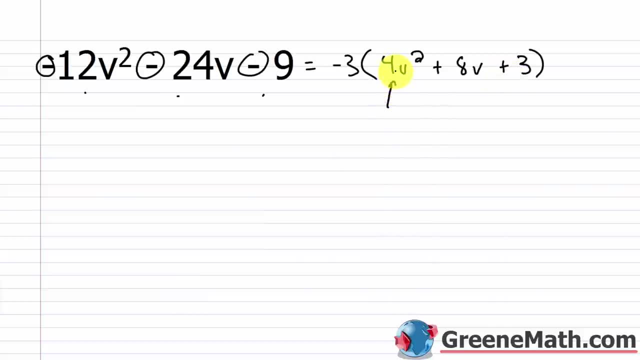 So again, I'm looking at the a or the coefficient for the squared term. And I'm looking for the c, which is the constant. So multiply those two together. 4 times 3 is 12. So product of 12. And then I'm looking for a sum of 8. So what are some factors of 12? We have 1 and 12. It's not going to work. We have 2 and 6. That would work. 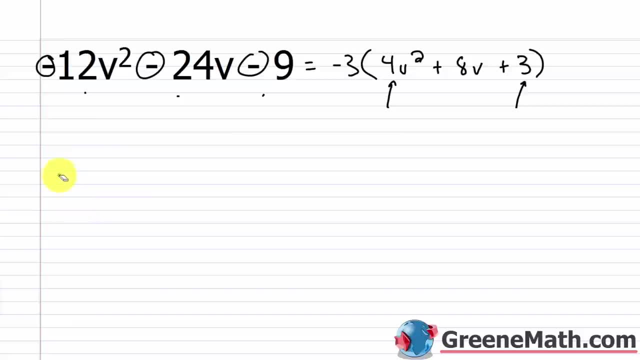 So let's rewrite that middle term. So we're going to have equals negative 3 times 4v squared. And I'm going to put plus 2v here. And then plus 6v here. Then plus 3. And then equals. 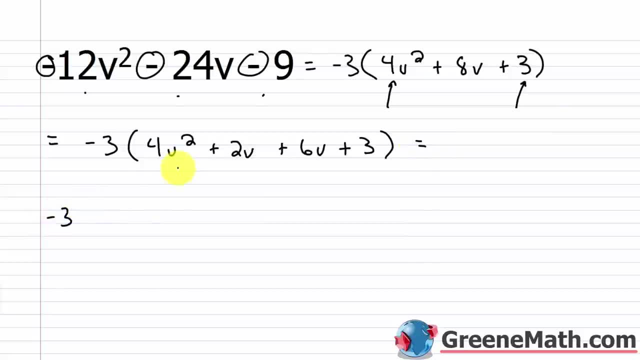 We'll put negative 3 out in front. We will break this up. 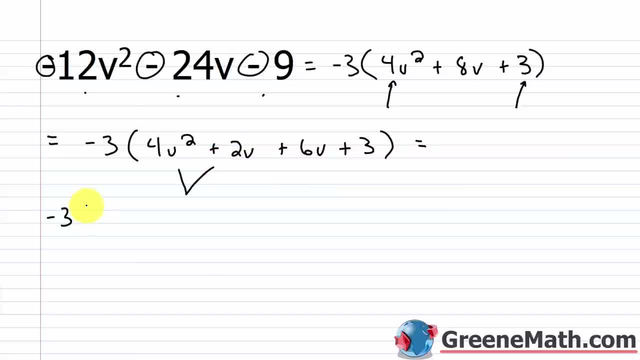 The greatest common factor here is 2v. So we'll put times. 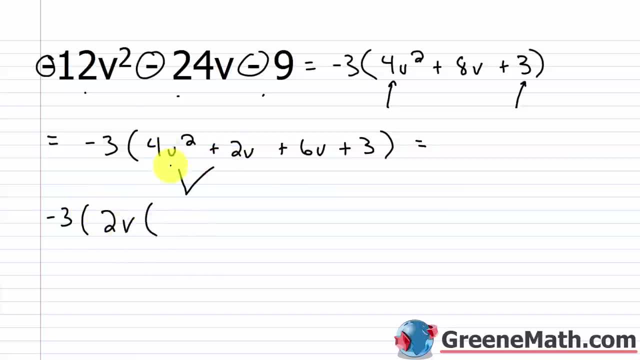 We'll have 2v times. Times. If I take that out, I'll have a 2v plus a 1. So then plus the GCF here is 3. So if I pull that out, I'll have a 2v plus a 1. 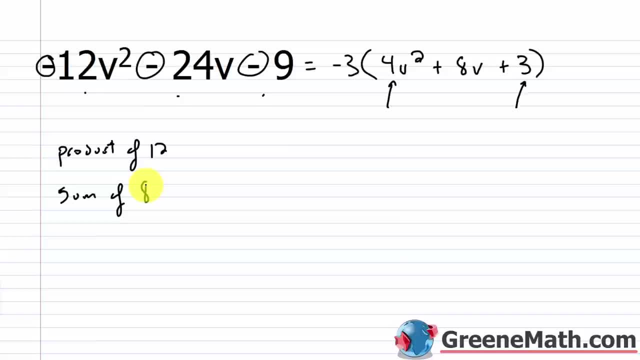 are some factors of 12. we have 1 and 12. it's not going to work. we have 2 and 6, that would work. so let's rewrite that middle term. so we're going to have equals negative 3 times 4 v squared and 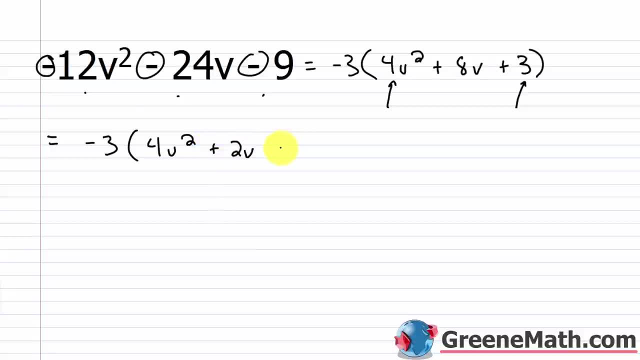 I'm going to put plus 2 v here, and then plus 6 v here, then plus 3 and then equals. we'll put negative 3 out in front. we will break this up. the greatest common factor here is 2 v, so we'll put: 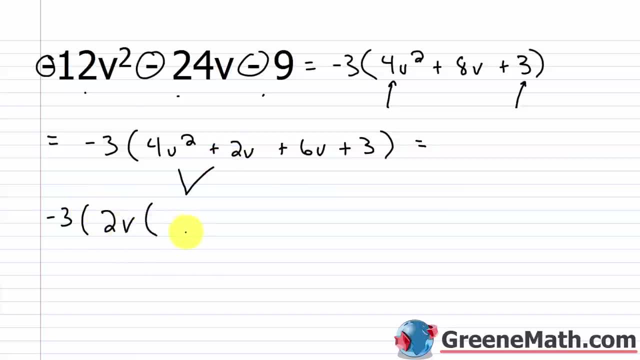 times, we'll have 2 v times. if I take that out, I'll have a 2 v plus a 1, so then plus the gcf here is 3. so if I pull that out, I'll have a 2 v plus a 1 and. 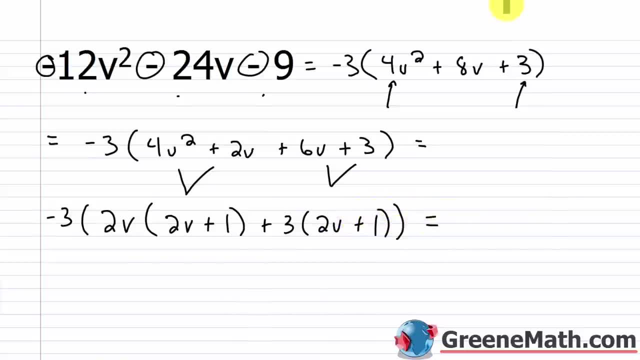 then if I factor out the common binomial factor here, that's 2 v plus 1, what am I going to have? I'll have a negative 3 out in front, and then I'll have 2 v plus 1, multiplied by 2 v plus. 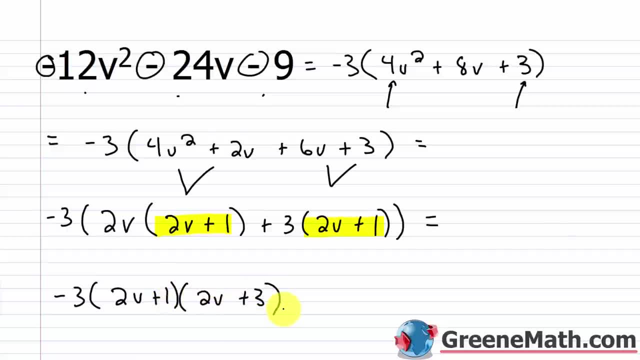 3. so there's my answer: negative 3 times 2 v plus 1 times 2 v plus 3. and again, you can check it in the interest of time. we still have a lot to cover. I'm not going to check it, but you should. 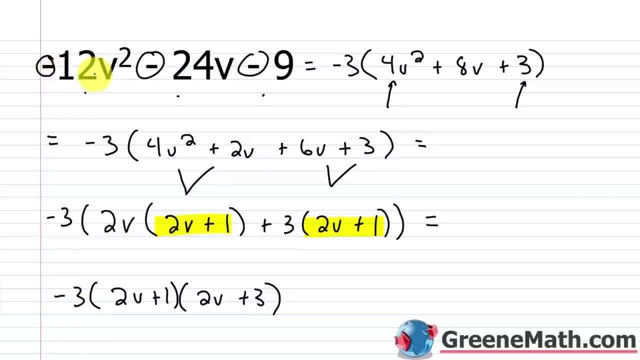 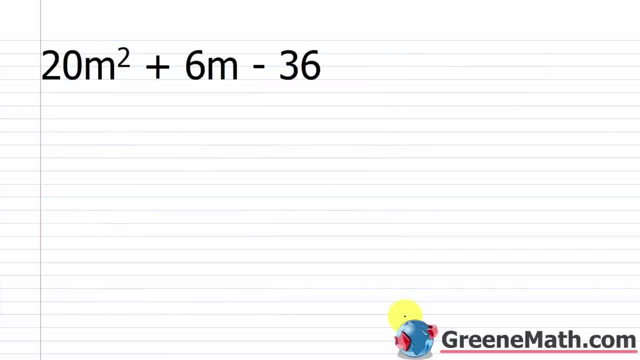 use FOIL for this and then multiply by negative 3 and you should get negative 12 v squared, minus 24 v minus 9 back as your answer. alright, let's take a look at one more and then we'll look at the reverse FOIL. 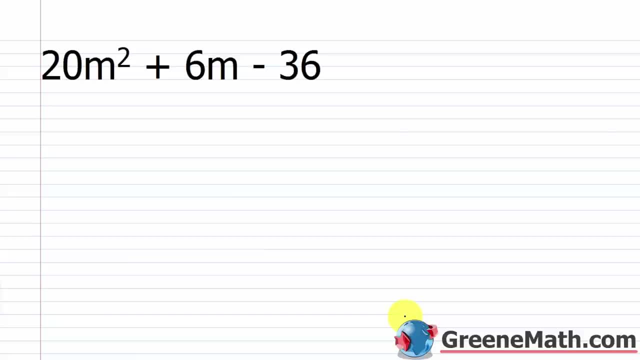 so we have 20 m squared plus 6 m minus 36, so everything is divisible by 2. so let's pull that out to start, so I'd have a 2 out in front and then 10 m squared plus 3 m minus 18. 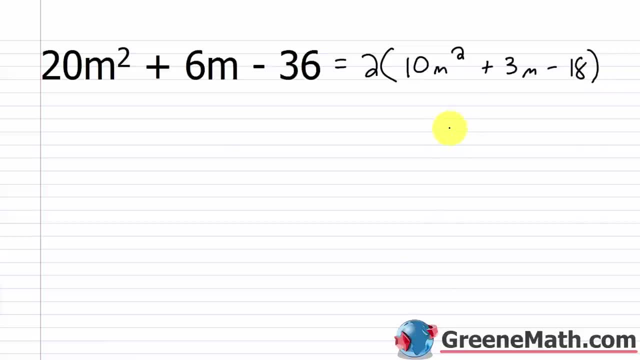 and then I'm looking at what's inside the parentheses here. so remember, I want a product of 10 times negative 18, that's negative 180 and a sum of 3. so we think about that. we know that we're going to have to have a positive and a negative. 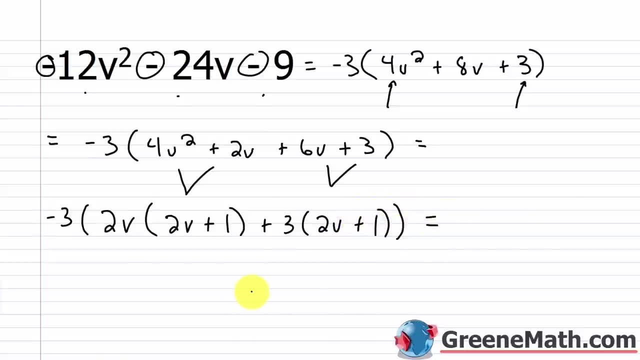 And then if I factor out the common binomial factor here, that's 2v plus 1. What am I going to have? I'll have a negative 3 out in front. And then I'll have 2v plus 1 multiplied by 2v plus 3. So there's my answer. 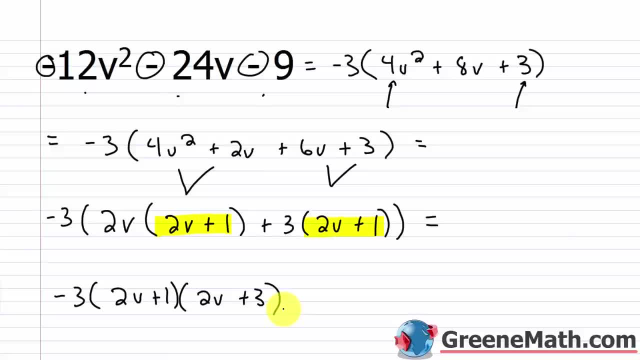 Negative 3 times 2v plus 1. 1 times 2v plus 3. And again, you can check it. In the interest of time, we still have a lot to cover. I'm not going to check it. But you should use FOIL for this and then multiply it by negative 3. 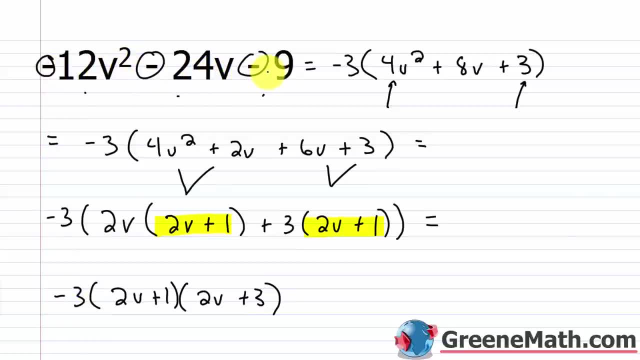 And you should get negative 12v squared minus 24v minus 9 back as your answer. All right. Let's take a look at one more. 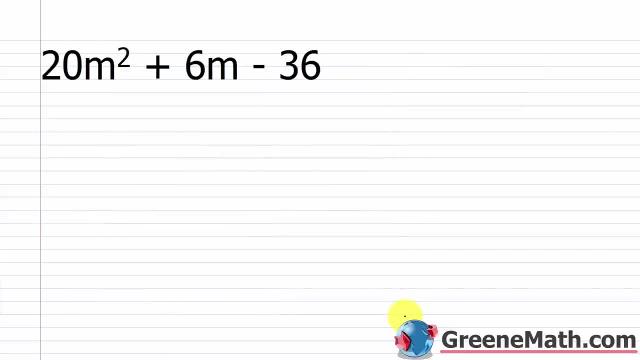 And then we'll look at the reverse FOIL. So we have 20m squared plus 6m minus 36. 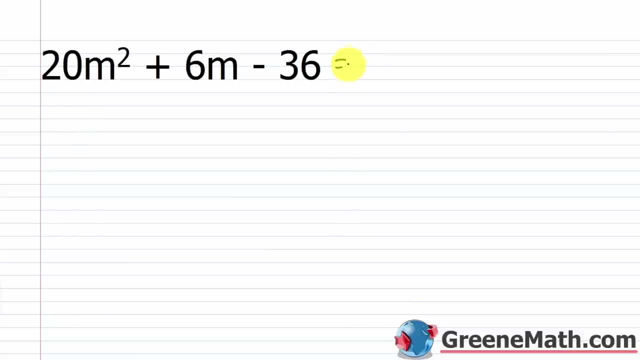 So everything is divisible by 2. So let's pull that out to start. So I'd have a 2 out in front. And then 10m squared. 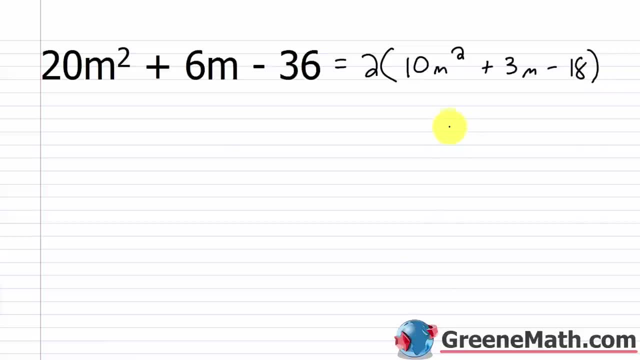 And then I'm looking at what's inside the parentheses here. So remember, I want a product of 10 times negative 18. That's negative 180. And a sum of 3. So we think about that. We know that we're going to have to have a positive and a negative. 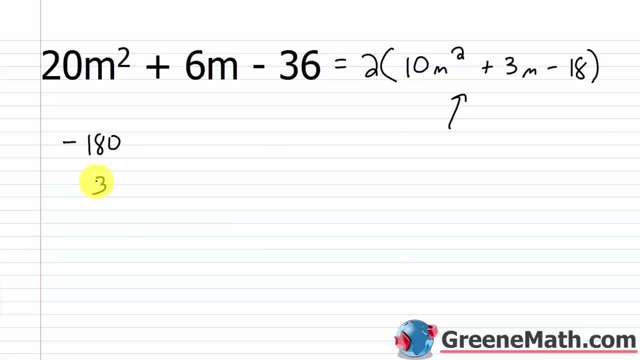 So what are some factors of 180? We've got 1 times 180. That's not going to work. You've got 2 times 90. That's not going to work. You've got 3 times 60. That's not going to work. You've got 4 times 45. Not going to work. 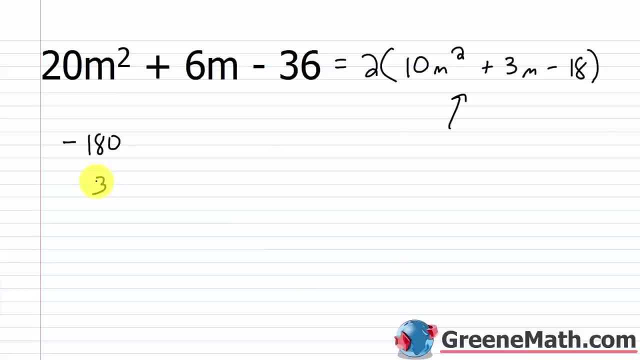 so what are some factors of 180? we've got 1 times 180, that's not going to work. you've got 2 times 90, that's not going to work. you've got 3 times 60, that's not going to work. you've got 4 times 45: not going to work. 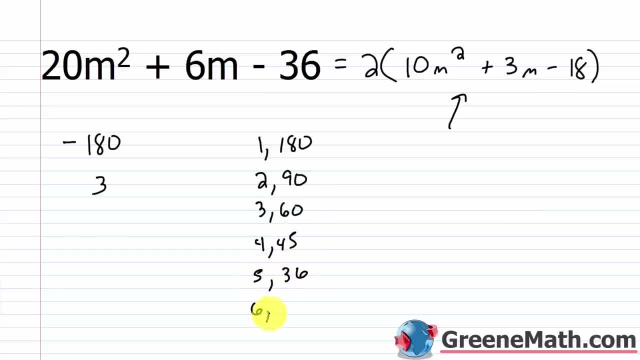 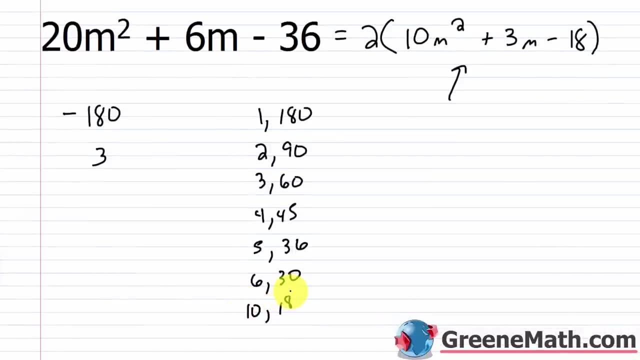 you've got 5 times 36 not going to work. you've got 6 times 30 not going to work and you've got 10 times 18. that's not going to work. what else do we have? we have 12 times 15. 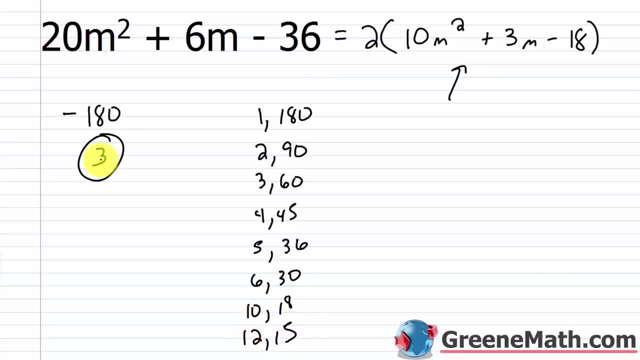 12 times 15 would work. for some way to work those signs out to where I can get 3 in my head, I just look at 12 and 15.. I know 15 minus 12 is 3.. So positive 15 and negative 12.. 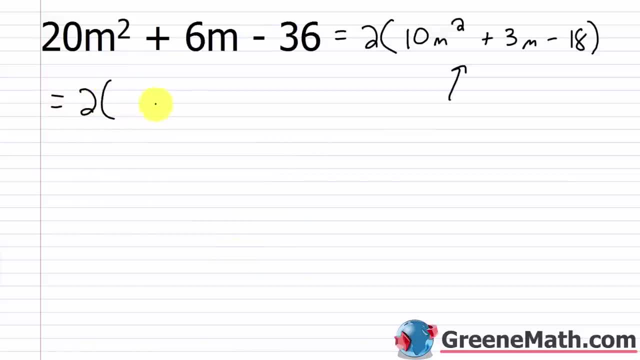 So let's rewrite this So we have 2 times, inside of parentheses, 10m squared. I'm going to rewrite that middle term, that 3m, as plus 15m and then minus 12m. All right, If I combine those together. 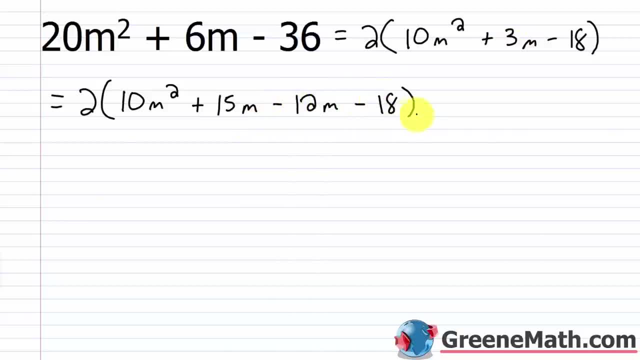 I get plus 3m and then minus 18.. Okay, So if I factor this by grouping I'll have 2 times inside of the parentheses Here. I would pull out from this first 2 a 5m, So 5m times 2m plus 3.. 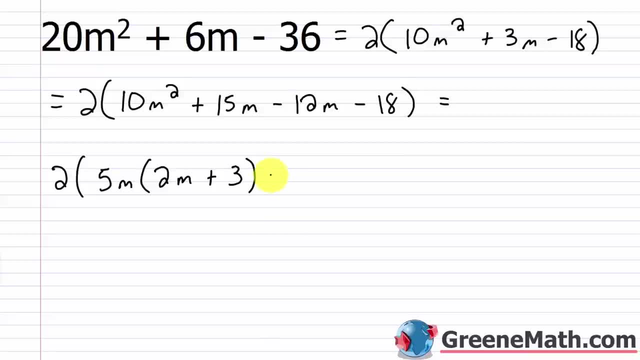 Then from this one we're going to pull out a negative 6. So minus 6 times you'd have 2m plus 3.. So my common binomial factor is 2m plus 3.. It's really easy to see. I can pull that guy. 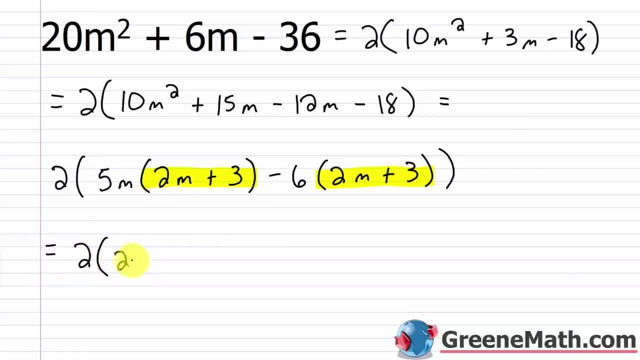 out. So I'd have 2 times 2m plus 3 times what's left. I'd have a 5m minus a 6.. So 2 times the quantity 2m plus 3 times 5m minus 6.. So again, if you want to check this, use FOIL here. 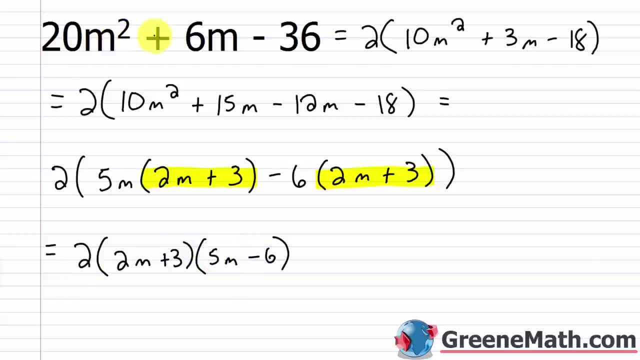 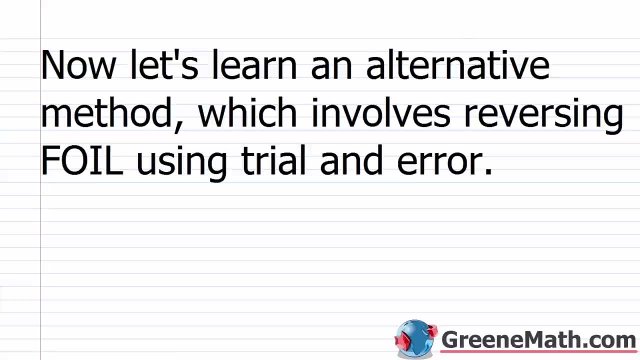 then multiply the result And you should get 20m squared plus 6m, minus 36 back. All right, So now let's learn an alternative method, which involves reversing FOIL using trial and error, And again, I just want to state that I 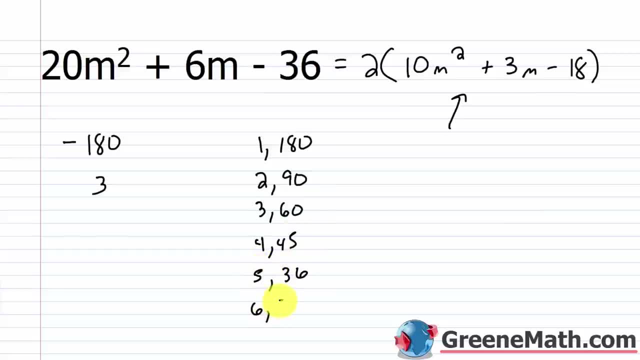 You've got 5 times 36. Not going to work. You've got 6 times 30. Not going to work. And you've got 10 times 18. That's not going to work. 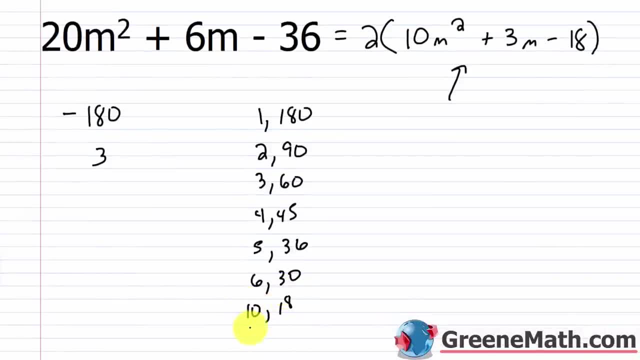 What else do we have? We have 12 times 15. 12 times 15 would work. 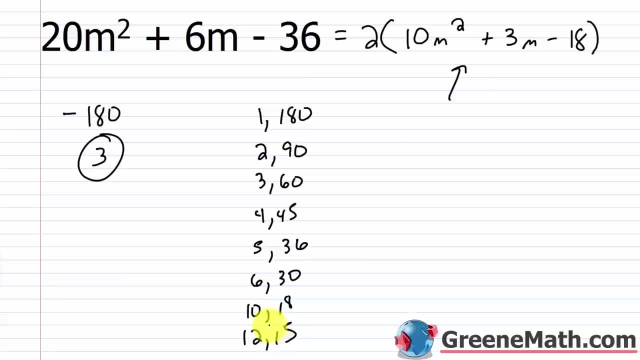 For some way to work those signs out to where I can get 3. In my head, I just look at 12 and 15. And I know 15 minus 12 is 3. 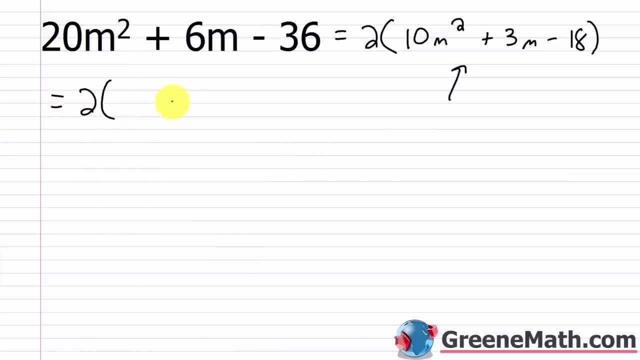 So let's rewrite this. So we have 2 times inside of parentheses 10m squared. I'm going to rewrite that middle term, that 3m, as plus 15m and then minus 12m. 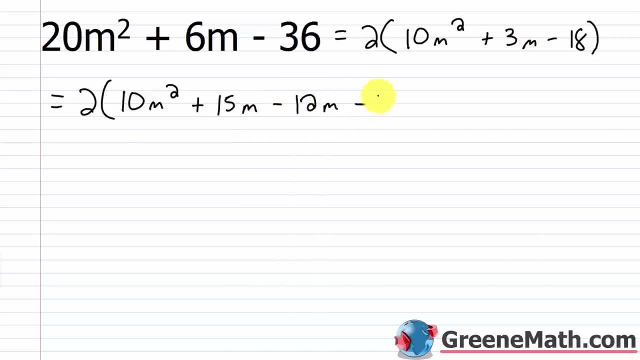 If I combine those together, I get plus 3m and then minus 18. Okay. 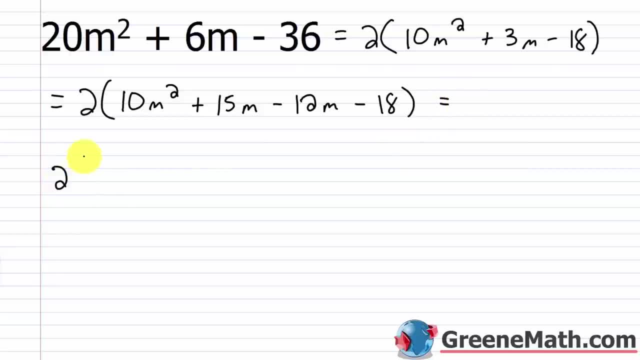 So if I factor this by grouping, I'll have 2 times inside of the parentheses. 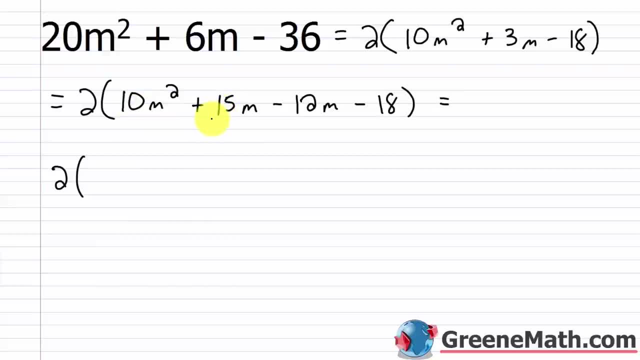 Here I would pull out from this first 2 a 5m. So 5m times 2m plus 3. 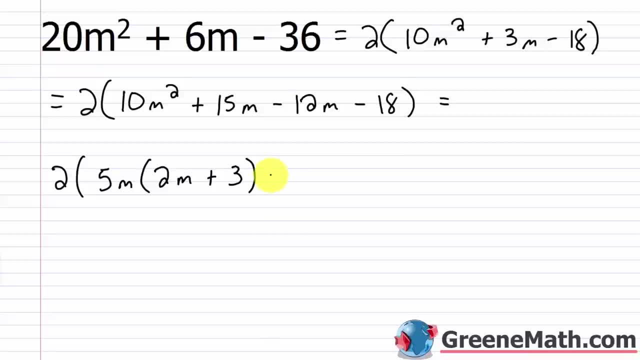 Then from this one, I'm going to pull out a negative 6. So minus 6 times, you'd have 2m plus 3. 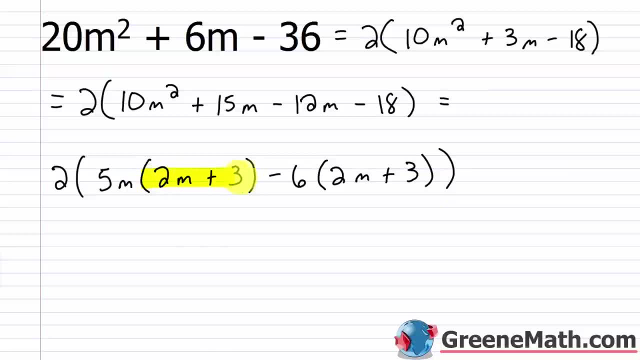 So my common binomial factor is 2m plus 3. It's really easy to see. I can pull that guy out. 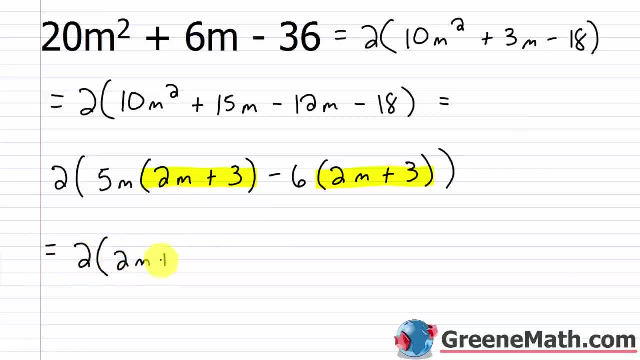 So I'd have 2 times 2m plus 3 times what's left. I'd have a 5m minus a 6. So 2 times the quantity 2m plus 3 times 5m minus 6. 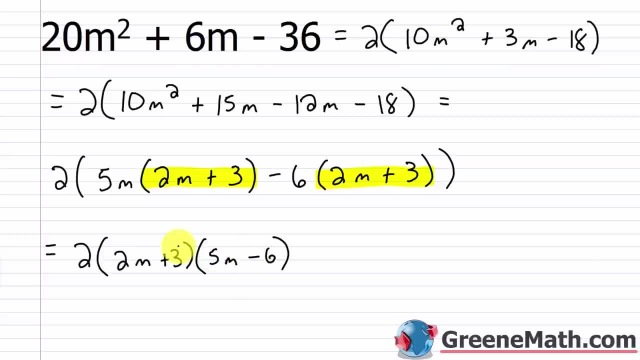 So again, if you want to check this, use FOIL here, then multiply the result by 2. And you should get 20m squared plus 6m minus 36 back. All right. So now, let's learn it all together. 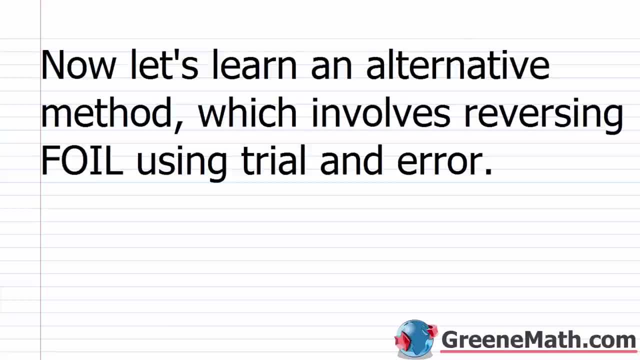 Let's learn an alternative method, which involves reversing FOIL using trial and error. And again, I just want to state that I personally don't like this method. 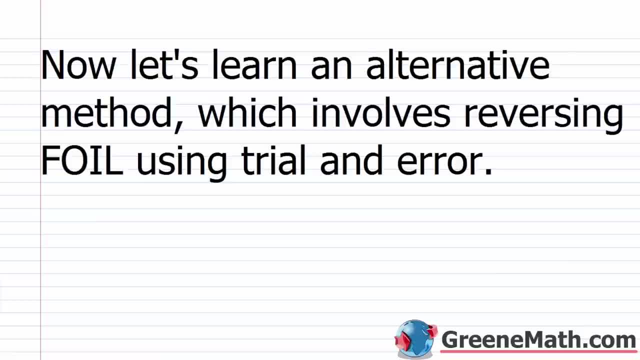 personally don't like this method. I don't use it. I find it to just be very tedious and very time consuming. I like using the factoring by grouping method, But for yourself, if you enjoy using this, if this is more productive for you. by all means, we're just trying to get. 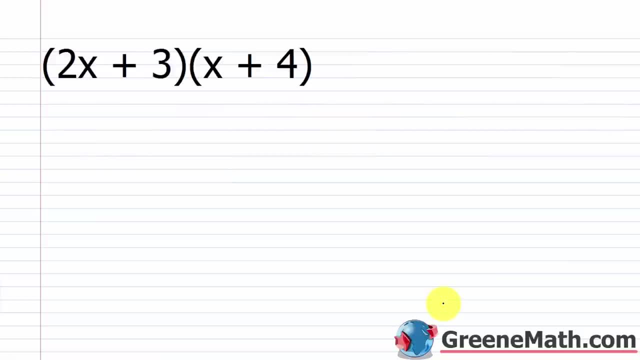 the correct answer In the end. All right, So I want to start out with just a demonstration of FOIL and then showing you how we would go about reversing this. So we know, FOIL is first term, So 2x times x is 2x squared. 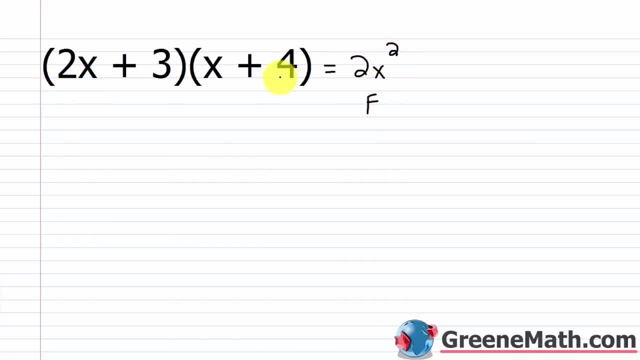 So this is the f. Then outer terms: 2x times 4 is plus 8x. This is the o. Then inner 3 times x is plus 3x. This is the i. And then last 3 times 4 is 12.. 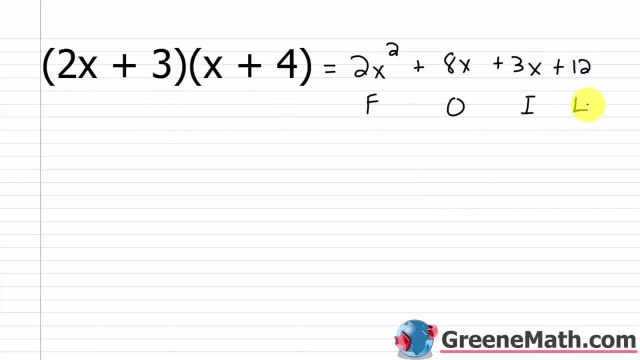 So plus 12.. This is last. So if we combine the outer and the inner, we're going to get a middle term that's 11x. So this is equal to 2x squared plus 11x plus 12.. Now what if I was to give you? 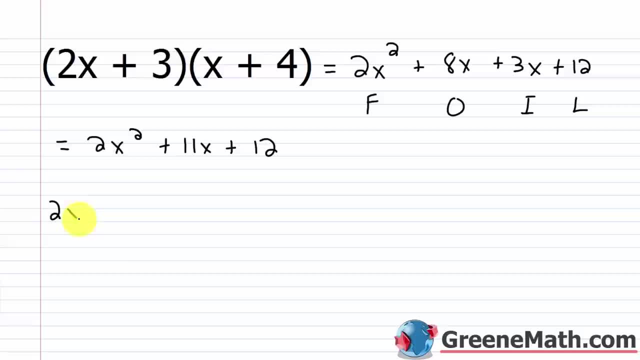 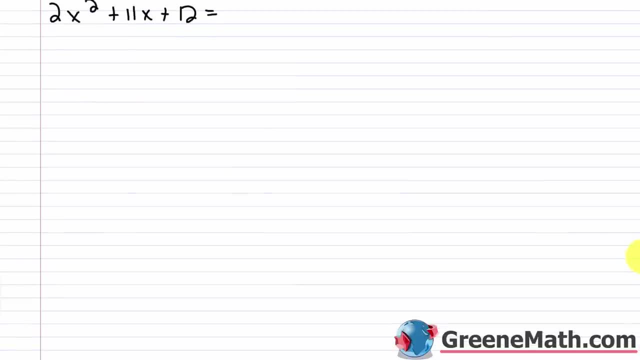 the 2x squared plus 11x plus 12, just like this. And I take this information away, So let's scroll down past it And cover it up And I tell you. I want you to factor this into the product of two binomials. 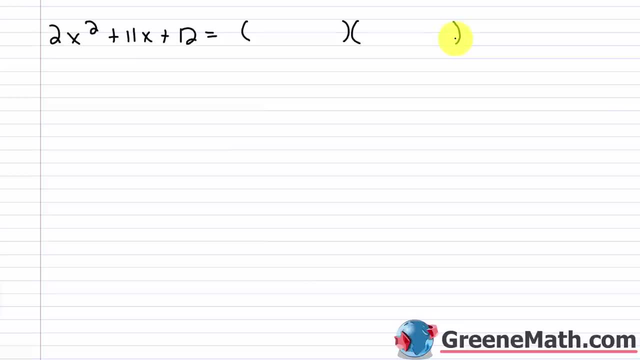 And I don't want you to use factoring by grouping. I want you to reverse the FOIL process. So the first thing is: let's think about FOIL, So we have the f. That's the first terms. So something times something gives me this guy right here, the 2x squared. So what are 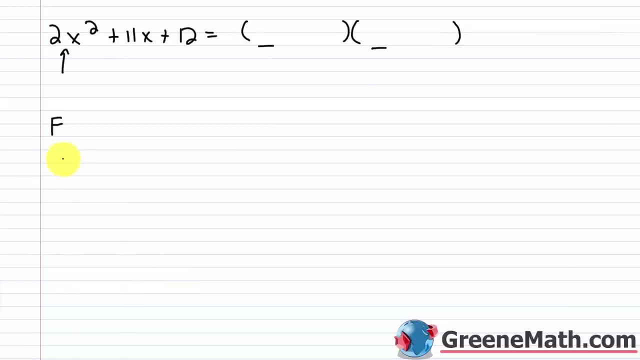 the possibilities for that. Well, since 2 is a prime number, really you can only do 2 times 1.. And x times x is x squared. So 2x times x is basically what you could do. Now you could consider negative 2x times. 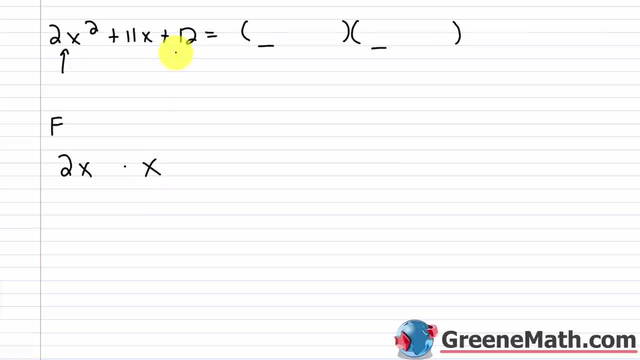 negative x, But everything is positive here, So you really don't need to think about that, You don't need to get that involved. You could say: or you know negative 2x times negative x, But we really don't need that And all the signs are positive. So if I just write, 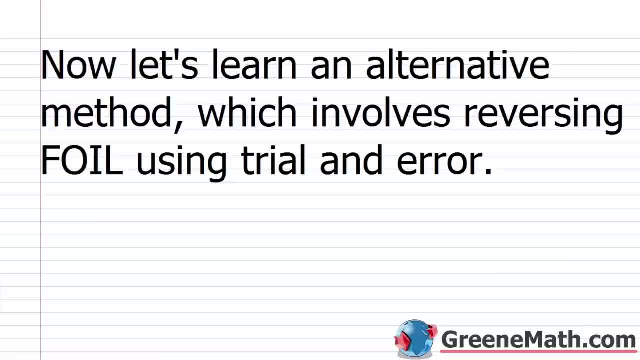 I don't use it. I find it to just be very tedious and very time-consuming. I like using the factoring by grouping method. But for yourself, if you enjoy using this, if this is more productive for you, you know, by all means, we're just trying to get the correct answer in the end. All right. 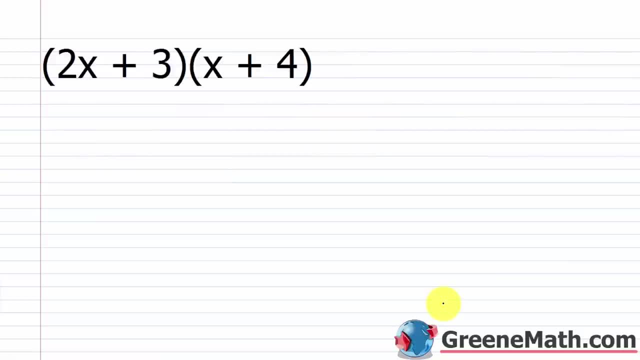 So I want to start out with just a demonstration of FOIL. And then show you how to do it. Okay. 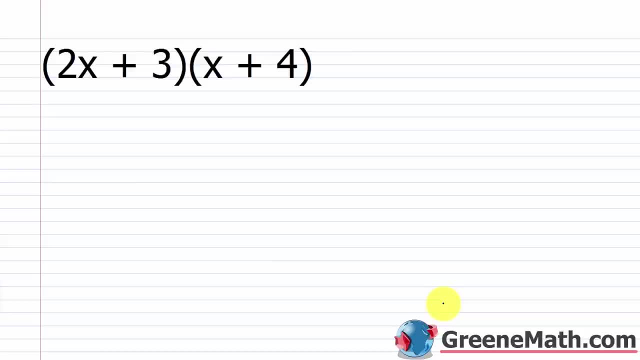 So let's get started. I'm going to be showing you how we would go about reversing this. So we know FOIL is first term. So 2x times x is 2x squared. So this is the F. Then outer terms, 2x times 4 is plus 8x. This is the O. Then inner, 3 times x is plus 3x. This is the I. And then last, 3 times 4 is 12. So plus 12. This is last. 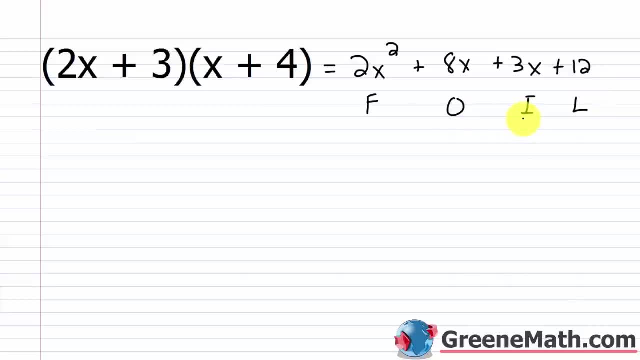 So if we combine the outer and the inner. We're going to get a middle term that's 11x. 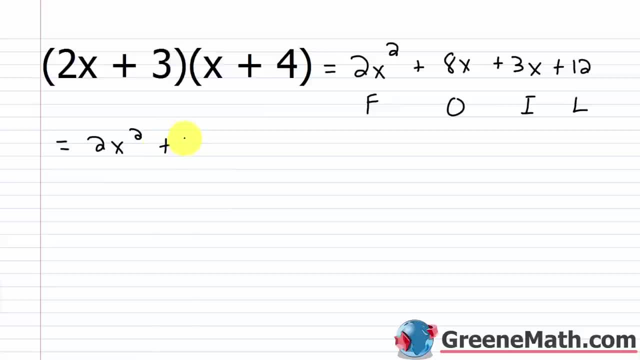 So this is equal to 2x squared plus 11x plus 12. 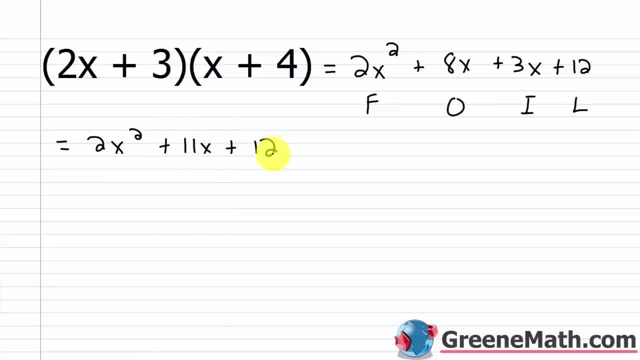 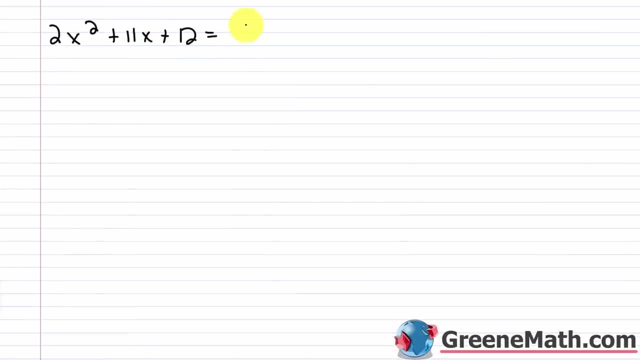 Now, what if I was to give you the 2x squared plus 11x plus 12, just like this. And I take this information away. So let's scroll down past it and cover it up. And I tell you, I want you to factor this into the product of two binomials, and I don't want you to use factoring by grouping. I want you to reverse the FOIL process. 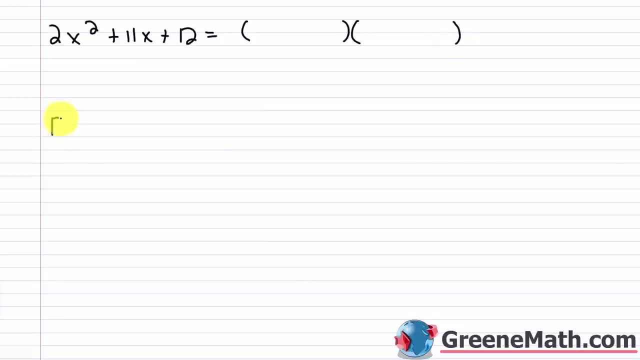 So the first thing is, let's think about FOIL. So we have the F. That's the first terms. So something times something gives me this guy right here, the 2x squared. So what are the possibilities for that? Well, since 2 is a prime number, really you can only do 2 times 1. And x times x is x squared. So 2x times x is basically what you could do. Now you could consider negative 2.5. You could consider negative 2.5. 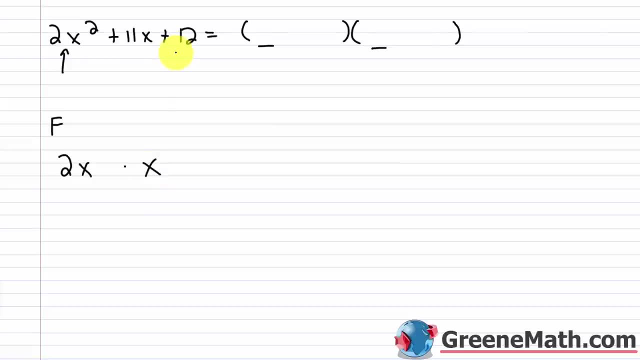 You could consider negative 2x times negative x. But everything is positive here, so you really don't need to think about that. 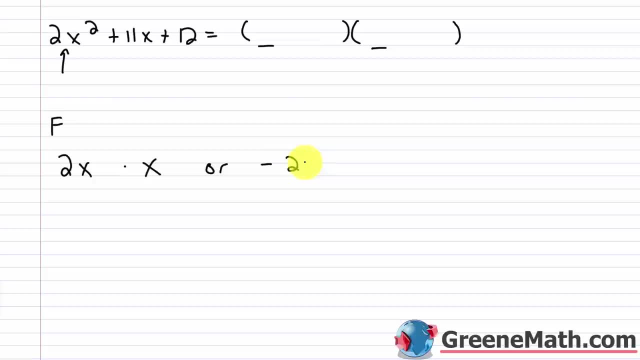 You don't need to get that involved. You could say OR negative 2x times negative x, but we really don't need that. 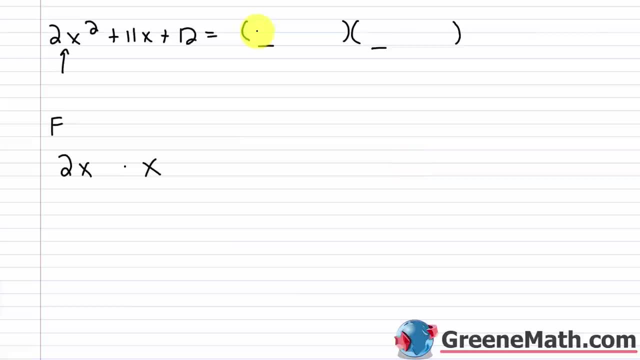 All the signs are positive. So if I just write out 2x times x like that, I know that 2x times x would give me 2x squared. So that's done. 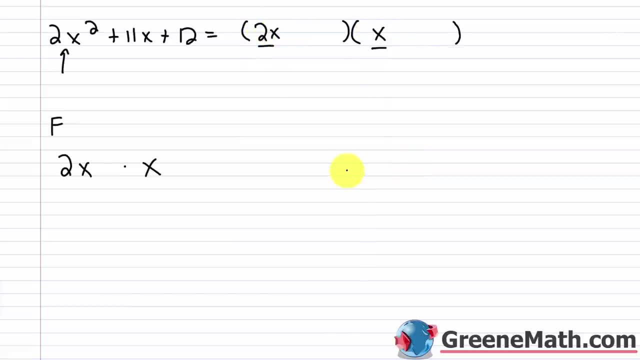 out 2x times x, like that. I know that 2x times x would give me 2x squared, So that's done. Now the next thing out would look at. I would skip the outer and the inner and I would look at the last, The last. 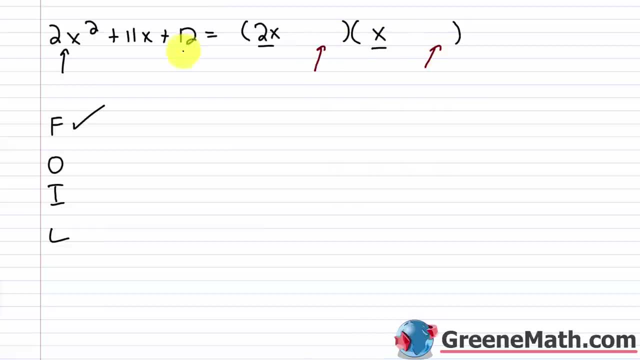 term here and the last term here will produce 12 when they're multiplied together. So I've got to go through all the factors of 12 and see what combination would give me a product of 12 and a sum of 11x. So that's where we talk about trial and error. For your factors of 12, you have 1. 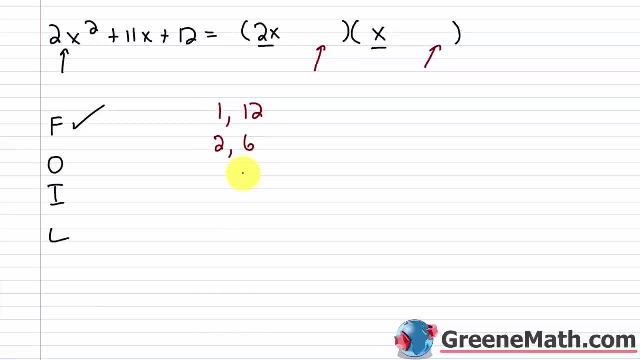 times 12,, you have 2 times 6, and you're going to have what? 3 times 4.. Now you have the negative versions of these: negative 1 times negative 12,. negative 2 times negative 6,, negative 3 times. 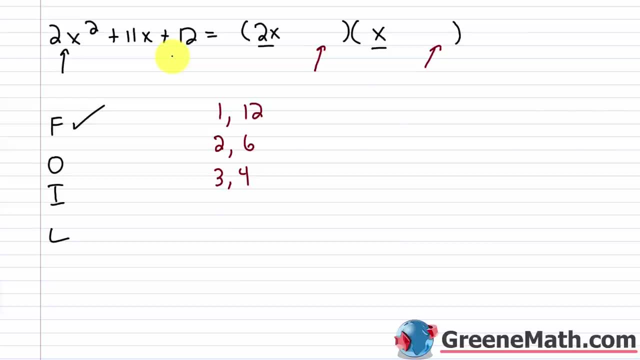 negative 4.. But again, all the signs are positive, so we don't really need to think about those at this point. So what I would do is I would go through again trial and error. You'd have let me put this down here: 1 times 12,, 2 times 6, and 3 times 4.. So let me make all the scenarios. 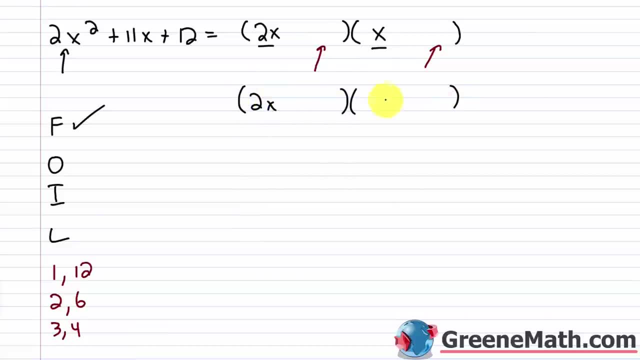 up. So you have 2x and x, and then you have 2x and x. So first I'm going to vary 1 and 12. Now I'm going to put plus 1 and plus 12.. So what I need to check here is the outer and the inner. Let me 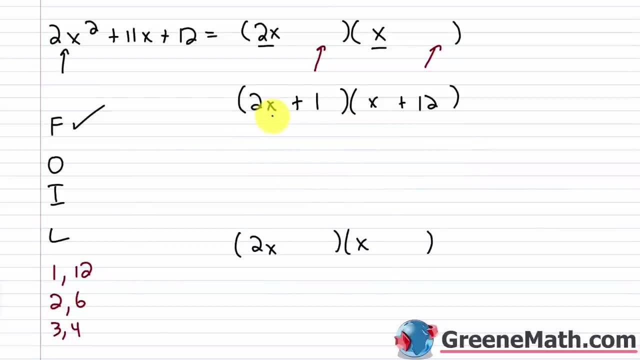 kind of move this down a little bit so I can show you that. So in other words, the outside here 2x times 12 is 24x. The inside here 1 times x is 1x If I combine like this: 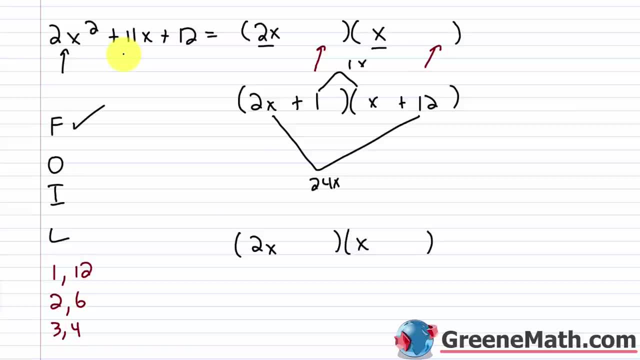 I can get 11x. So the answer to that is no. So that's not going to be my solution, So I would start with something else then. Now I could reverse the order here and try 12 and then try 1,. 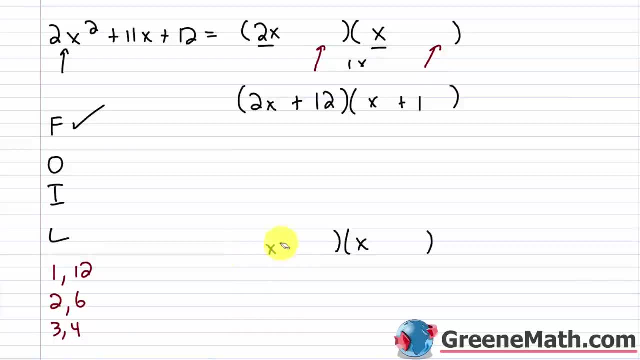 but there's one little tip that I want to give you. If your original trinomial did not have a common factor, then you're not going to have a common factor in any of the binomials. So in other words, this has a common factor of 2.. I could pull a 2 out and I'd have x, y and z. So 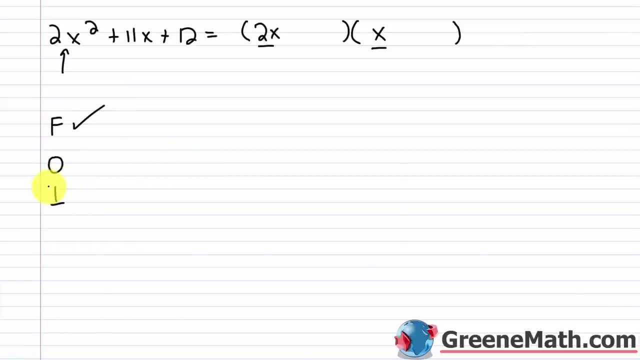 Now the next thing I would look at, I would skip the outer and the inner, and I would look at the last. 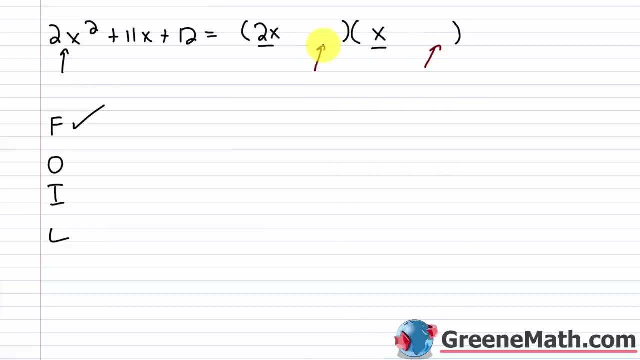 The last term here. The last term here. And the last term here will produce 12 when they're multiplied together. 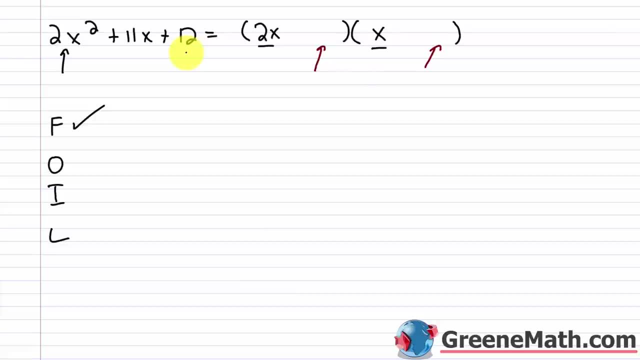 So I've got to go through all the factors of 12 and see what combination would give me a product of 12 and a sum of 11x. 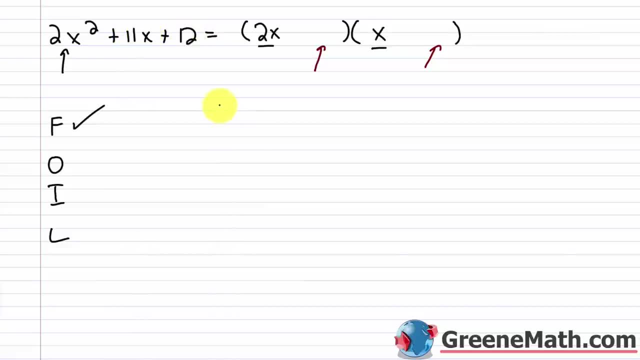 So that's where we talk about trial and error. For your factors of 12, you have 1 times 12. You have 2 times 6. And you're going to have what? 3 times 4. Now. 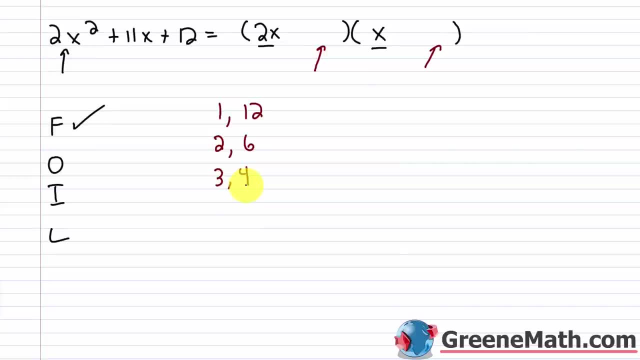 You have the negative versions of these. Negative 1 times negative 12. Negative 2 times negative 6. Negative 3 times negative 4. 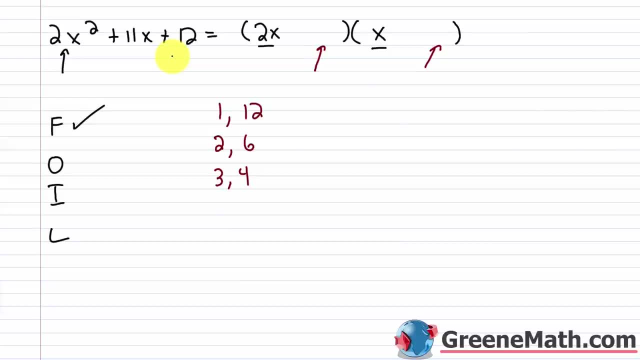 But again, all the signs are positive, so we don't really need to think about those at this point. 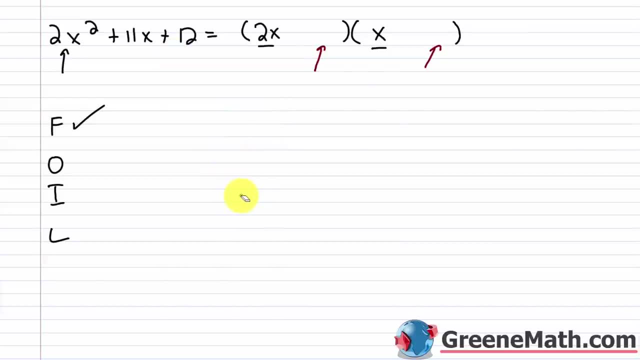 So what I would do is, I would go through, again, trial and error. You'd have, let me put this down here, 1 times 12, 2 times 6, and 3 times 4. 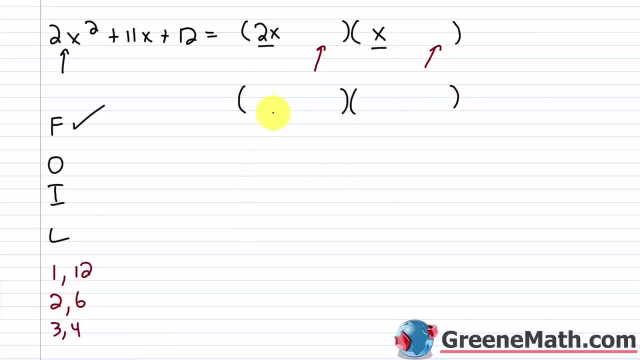 So let me make all the scenarios up. So you have 2x and x. 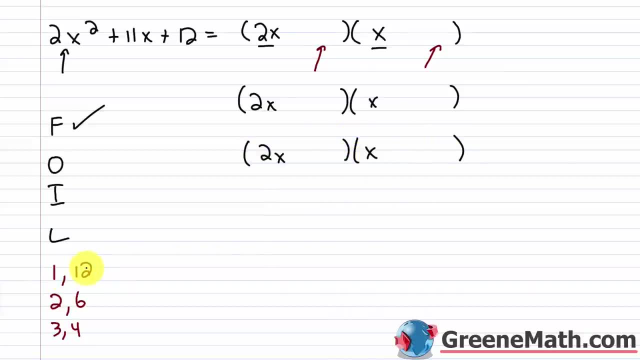 So first I'm going to. So first I'm going to vary 1 and 12. 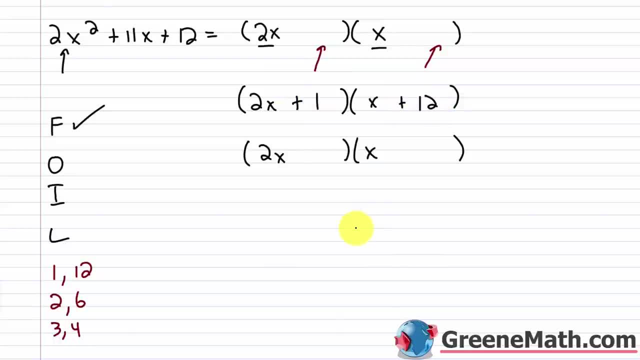 Now I'm going to put plus 1 and plus 12. So what I need to check here is the outer and the inner. Let me kind of move this down a little bit so I can show you that. So in other words, the outside here, 2x times 12 is 24x. 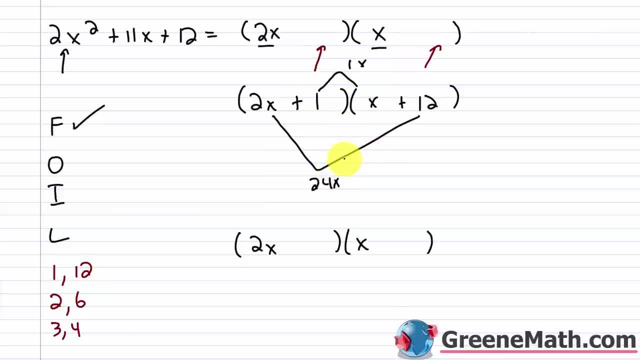 The inside here, 1 times x is 1x. If I combine like terms with that, would I get 11x? 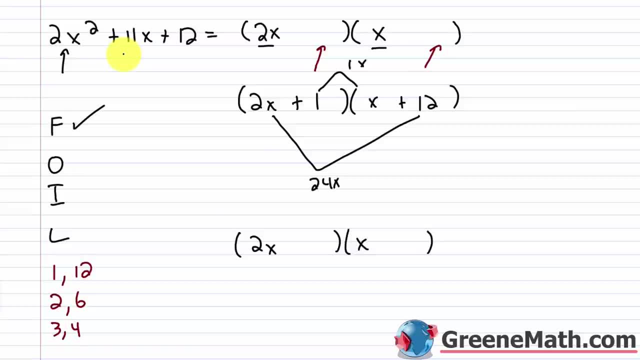 The answer to that is no. So that's not going to be my solution. 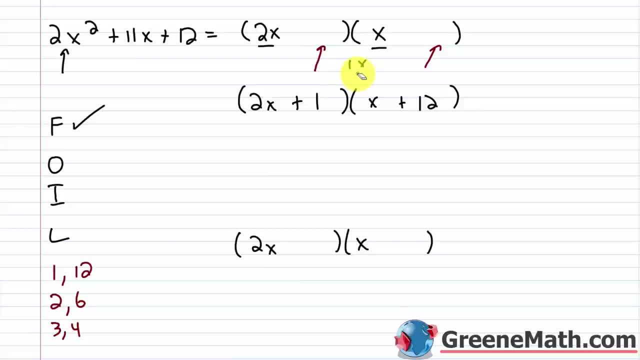 So I would start with something else then. Now I could reverse the order here and try 12 and then try 1. 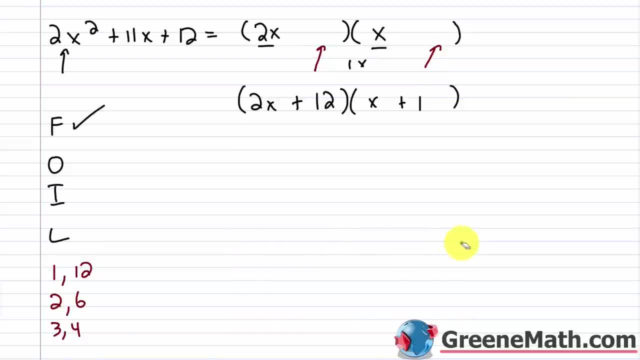 But there's one little tip that I want to give you. If your original trinomial did not have a common factor, then you're not going to have a common factor in any of the binomials. 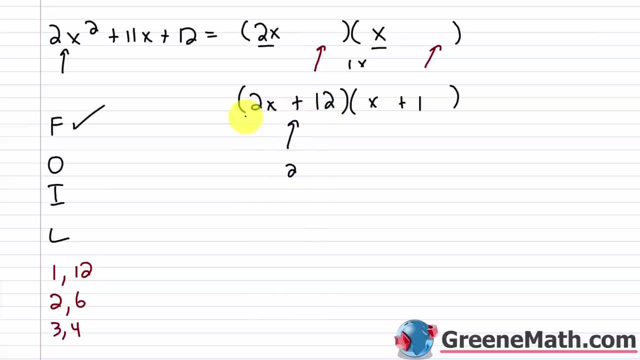 So in other words, this has a common factor of 2. I could pull a 2 out and I'd have x plus 6. 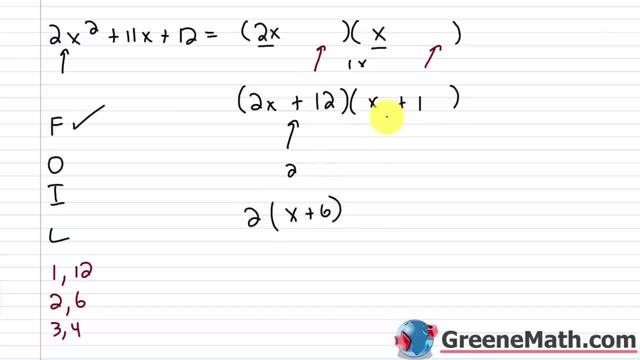 this isn't a possibility, So we can eliminate that, And once we've eliminated that, we can cross this one off the list. That's not going to work, So now let's try 2 and 6.. Now, if I put 2, 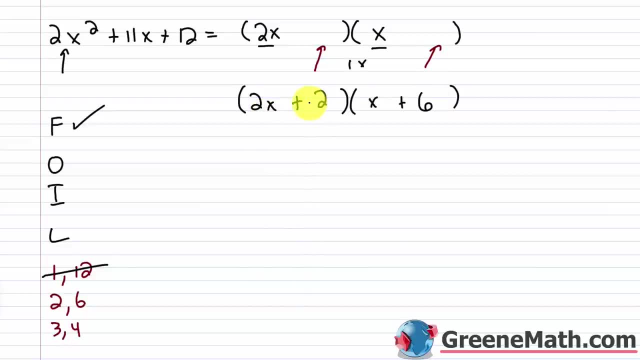 here and 6 here, again there's a common factor of 2.. So that's not going to work. So if I switch that up and put 6 here and 2 here, common factor of 2, that's not going to work. So that's. 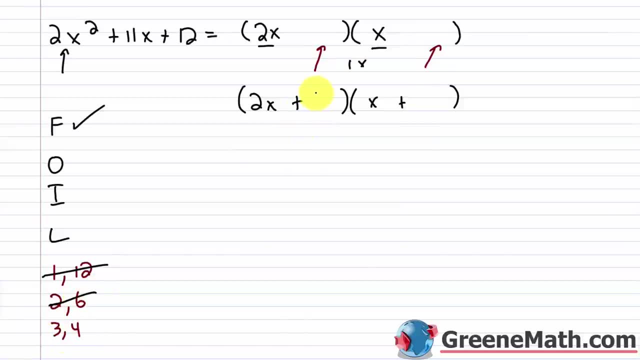 eliminated, So now I'm just down to 3 and 4.. So I can put 3 here and 4 here and try that. So the outer 2x times 4 would be 8x. The inner 3 times x would be 3x If I add those two together. 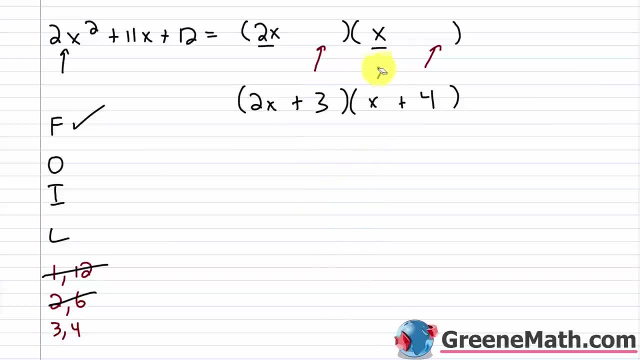 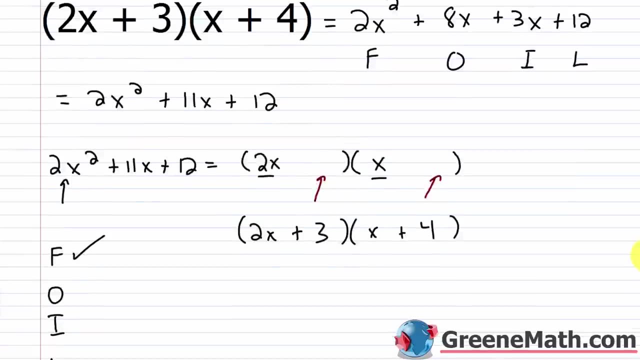 8x plus 3x is 11x. So here's my factored form. I have 2x plus 3 times x plus 4, those two quantities, And we know that because we did this problem earlier. right, We saw it from kind of. 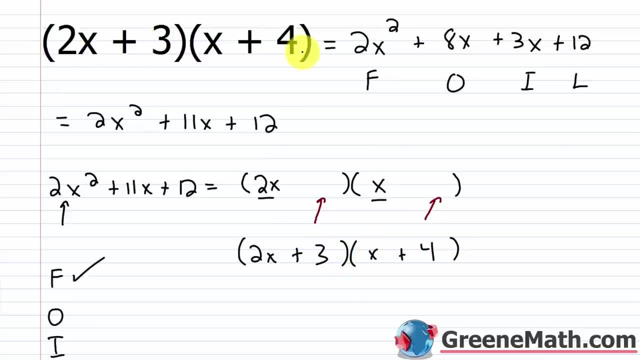 this form: 2x plus 3,, 2x plus 3,, x plus 4, and x plus 4.. So you can see that's a lot more tedious, a lot more involved. I'm going to give you an easy scenario. right, The coefficient on the x squared term is a prime. 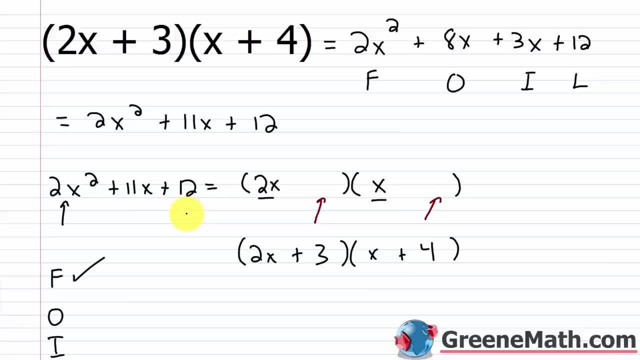 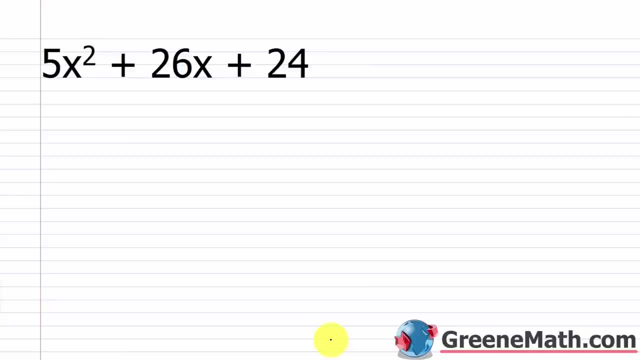 number and everything is positive. So we have a lot less work with this versus another scenario which would be more complex. Okay, let's take a look at 5x squared plus 26x plus 24.. So, again, I'm going to set this up as the product of two binomials there. 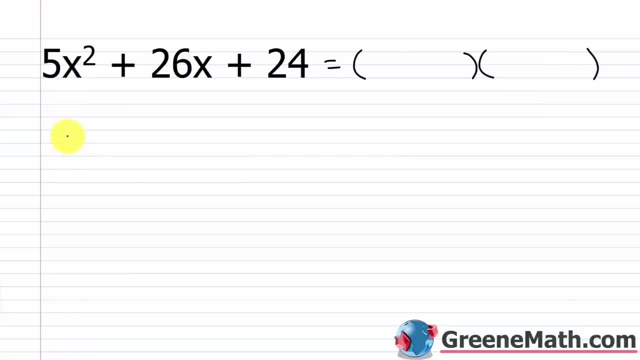 And for 5, that's a prime number. So I'm thinking about what 5x times x? again, everything is positive, So I really don't need to think about negative 5x times negative x. I don't need to involve that, So I'm just going to start out with 5x times x. That's for the first. 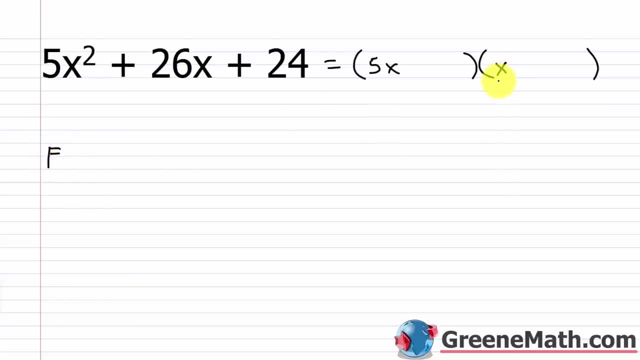 part of FOIL right F. So that's what that comes from. Now I'm going to do the L. So for 24, something times something, it's got to give me 24.. So what are the factors of 24?? Well, 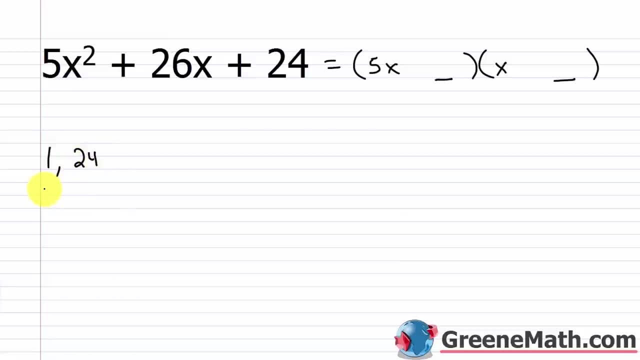 I've got what? I've got 1 times 24.. I've got 2 times 24.. I've got 2 times 24.. I've got 2 times 24.. I've got 3 times 8.. I've got 4 times 6.. And then that's going to be it. So if I start with 1 times, 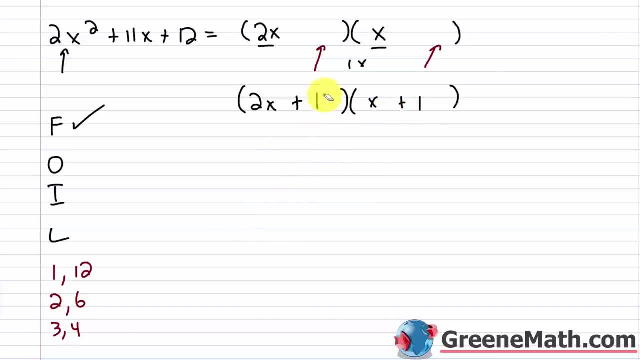 So this isn't a possibility. So we can eliminate that. And once we've eliminated that. We can cross this one off the list. That's not going to work. 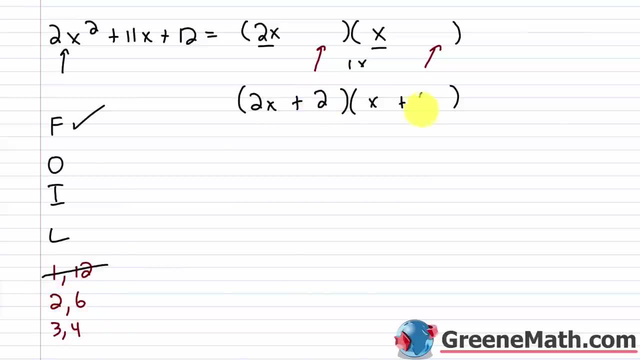 So now let's try 2 and 6. Now if I put 2 here and 6 here, again there's a common factor of 2. 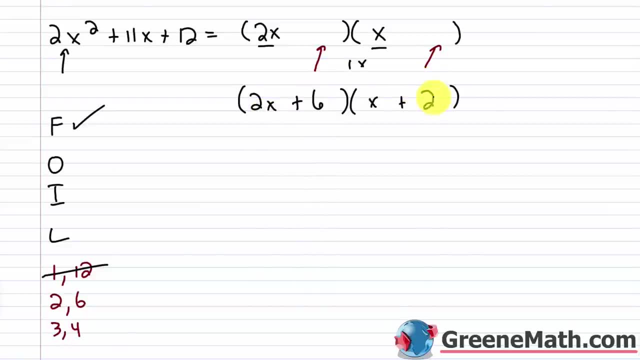 So that's not going to work. So if I switch that up and put 6 here and 2 here, common factor of 2, that's not going to work. 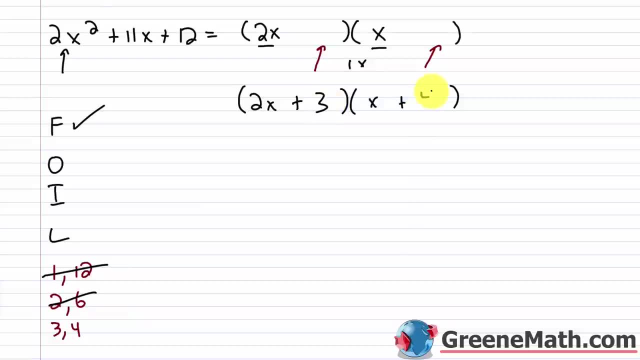 So now I'm just down to 3 and 4. So I can put 3 here and 4 here and try that. So the outer, 2x times 4 would be 8x. The inner, 3 times x would be 3x. If I add those two together, 8x plus 3x is 11x. So here's my factored form. 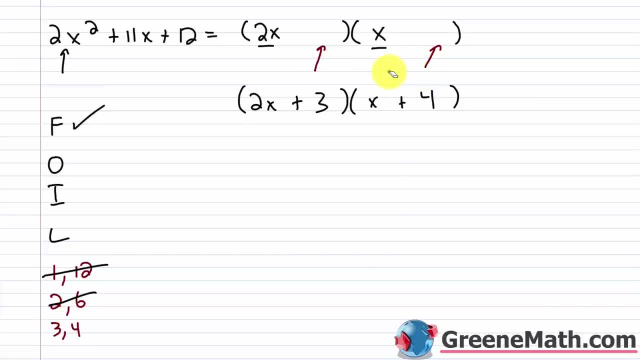 I have 2x plus 3 times x plus 4. Those two quantities. And we know that because we did this problem earlier. 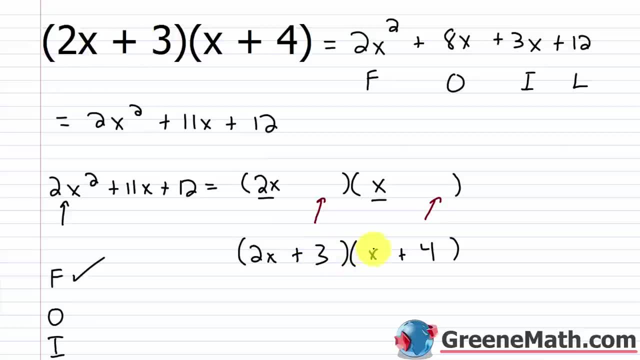 We saw it from kind of this form, 2x plus 3, 2x plus 3, x plus 4, and x plus 4. So you can see that's a lot more tedious, a lot more involved. And I gave you an easy scenario, right? The coefficient on the x squared term is a prime number. And everything is positive. 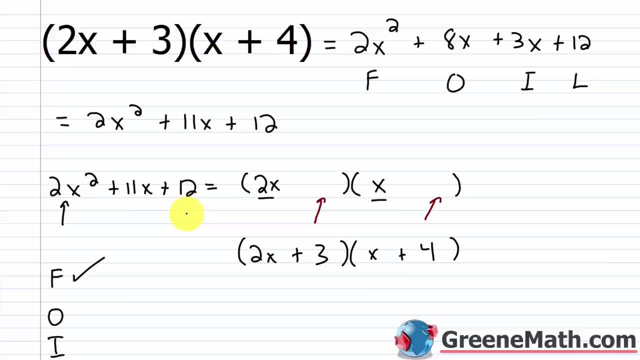 So we have a lot less work with this versus another scenario, which would be more complex. 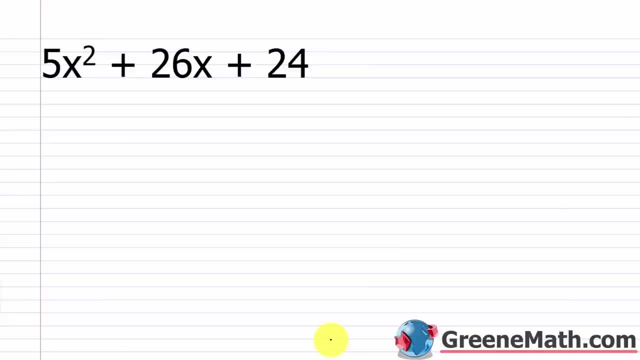 Okay, let's take a look at 5x squared plus 26x plus 24. So again, I'm going to set this up as the product of two binomials there. And for 5, that's a prime number. So I'm thinking about what, 5x times x. Again, everything is positive. So I really don't need to think about negative 5x times negative x. I don't need to involve that. So I'm just going to start out with 5x times x. 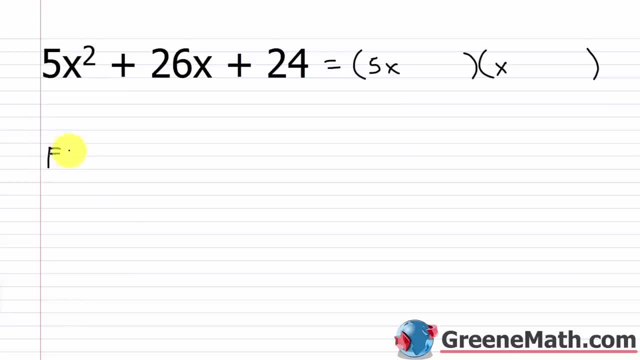 That's for the first part of FOIL, right, F. So that's what that comes from. 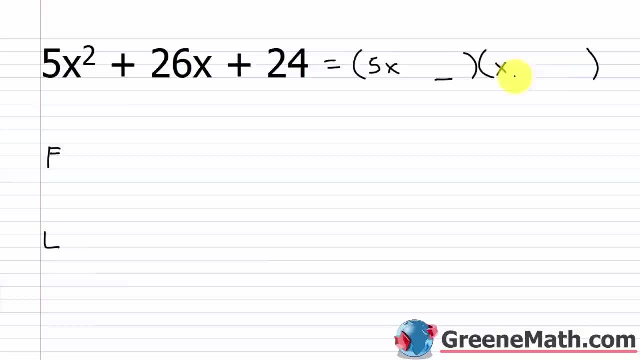 Now I'm going to do the L. So for 24, something times something has got to give me 24. So what are the factors of 24? Well I've got what? I've got 1 times 24. I've got 2 times 12. I've got 3 times 8. I've got 4 times 6. And then that's what I'm going to do. Okay. So that's going to be it. 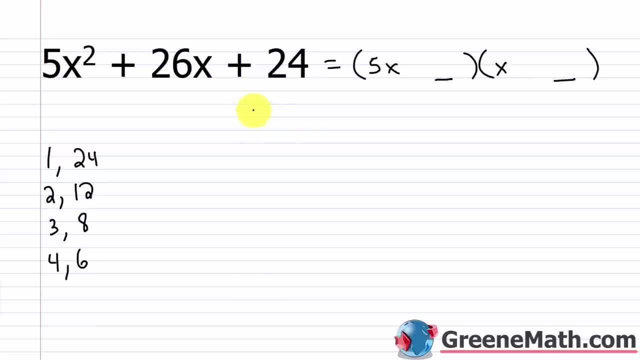 So if I start with 1 times 24, let me kind of look at these scenarios here. So 5x and x, let me make out a few different scenarios. So I've got positive 1, positive 1, positive 24, and positive 24. And then I'll check 2 and 12 also. So plus 2, plus 12. Plus 12. Plus 12. 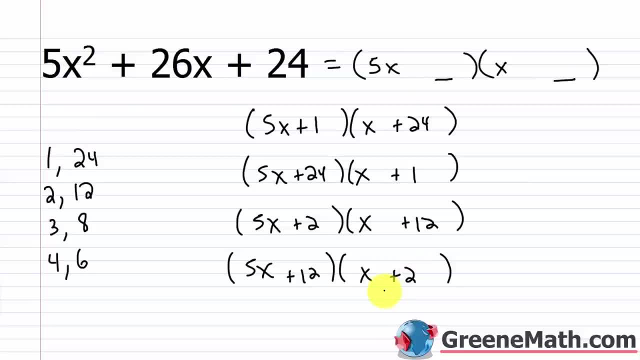 And plus 2. So you can kind of set it up like this and check it very quickly. 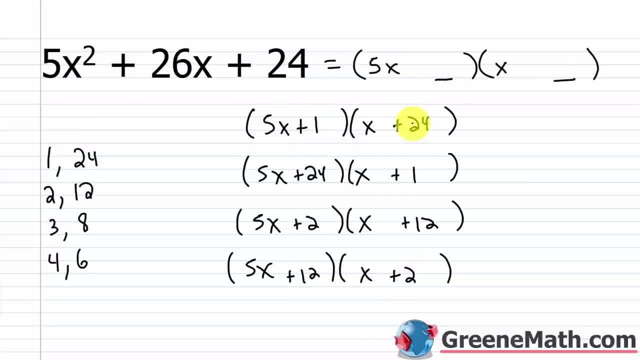 So all you're looking at is the outer. So forget about the x for a second. 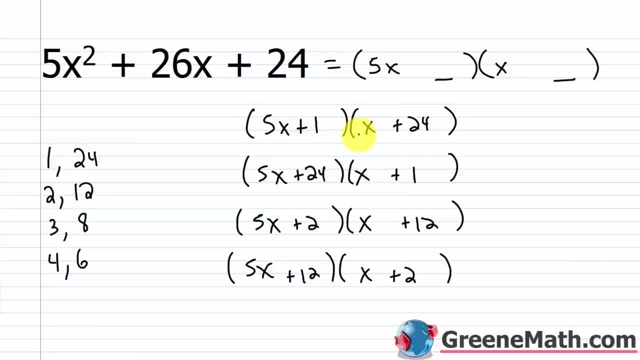 5 times 24 is 120. The inner would be 1. So 120 plus 1 is 121. That's not going to get you to 26. The outer here, 5 times 1 is 5. 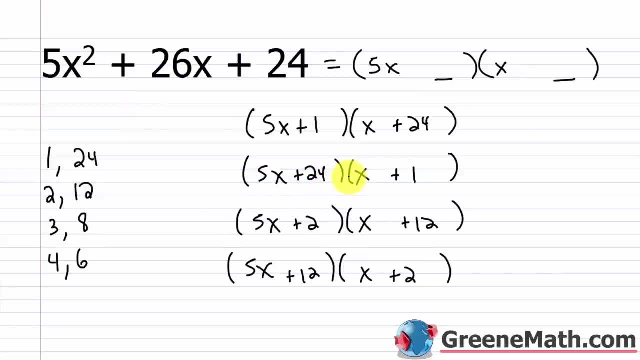 The inner, 24 times 1 is 24. 5 plus 24 is 29. So that's not going to work. So this one is eliminated. 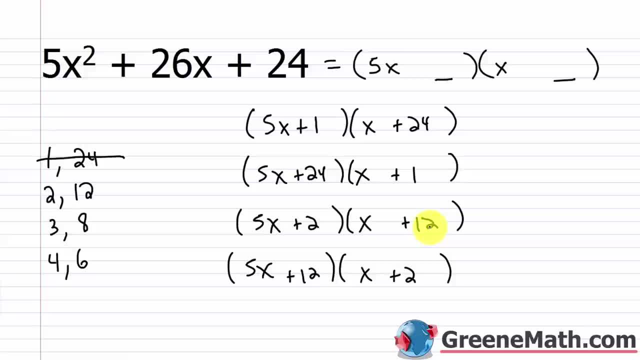 Then for this one, 5 times 24. 5 times 12 is 60. The inside, 2 times 1 is 2. So that's 62. That's not going to work. 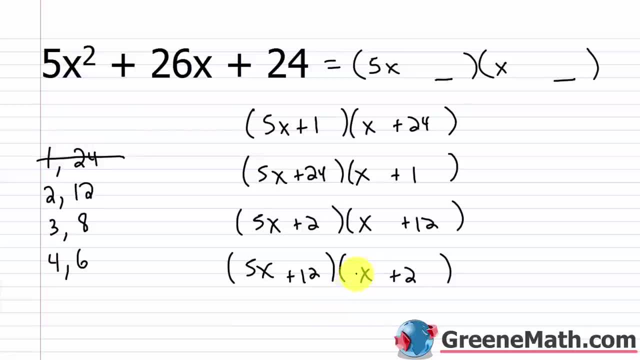 5 times 2 is 10. 12 times 1 is 12. 10 plus 12 is 22. 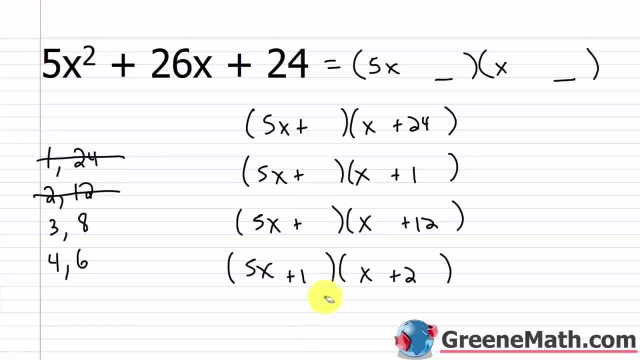 So that's not going to work. So you can get rid of all of those scenarios. None of those work. 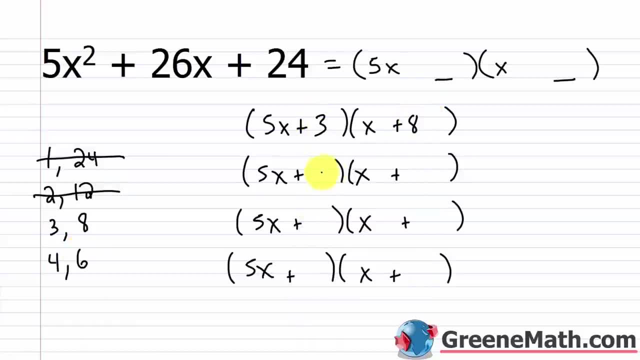 And now we can go on to 3 and 8. And let's try 4 and 6 if we need to. Okay. So 5 times 8 is 40. 3 times 1 is 3. 43 is not going to work. 5 times 3 is 15. 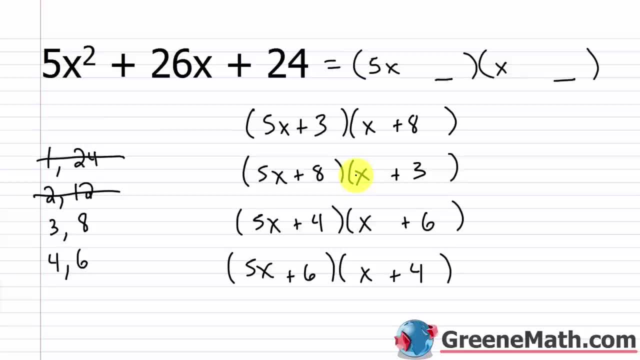 And then 8 times 1 is 8. 15 plus 8 is 23. That's not going to work. So this is eliminated. So now I'm down to the last possibility. 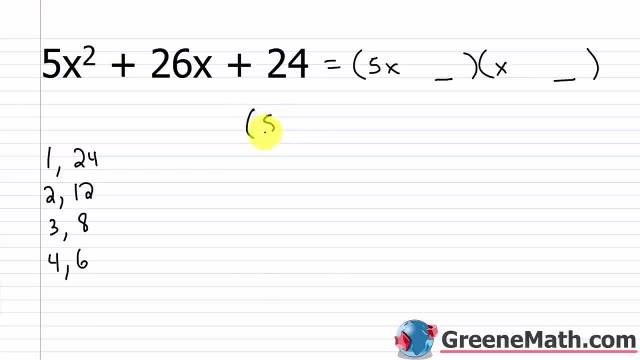 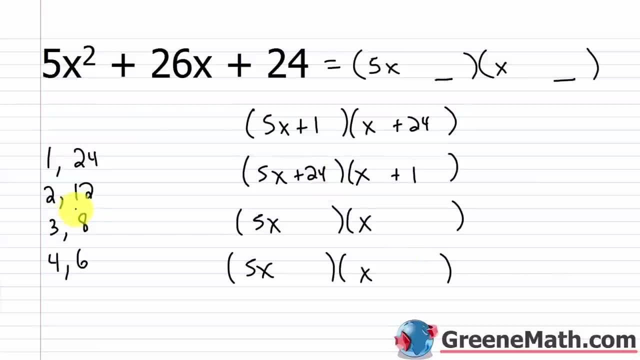 positive 24, and positive 24.. And then I'll check 2 and 12 also. So plus 2,, plus 12,, plus 12, and plus 2.. So you can kind of set it up like this and check it very quickly. So all you're looking. 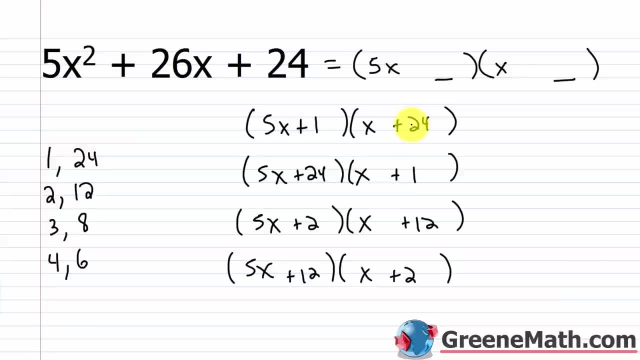 at is the outer, So forget about the x for a second. 5 times 24 is 120.. The inner would be 1.. So 120 plus 1 is 121.. That's not going to get you to 26.. The outer here, 5 times 1 is 5.. The inner: 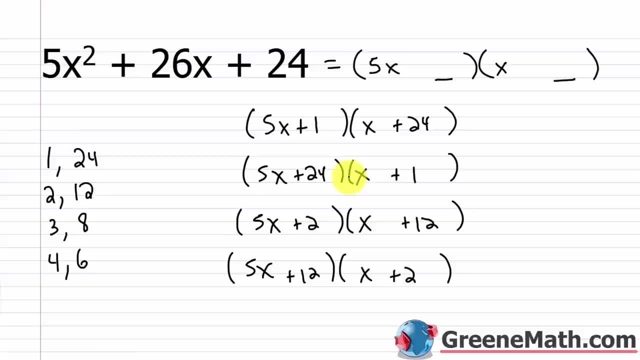 24 times 1 is 24.. 5 plus 24 is 29.. So that's not going to work. So this one is eliminated. Then for this one, 5 times 12 is 60. The inside 2 times 1 is 2.. So that's 62. That's not going to work. 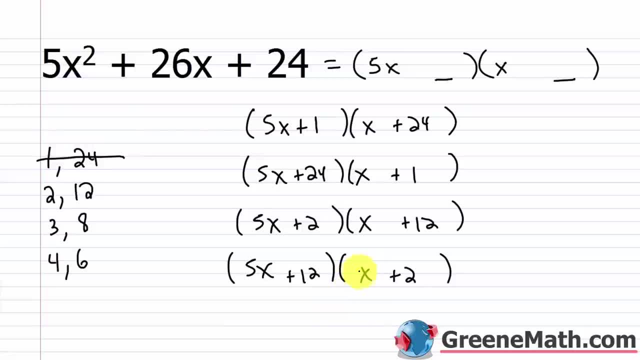 5 times 2 is 10.. 12 times 1 is 12.. 10 plus 12 is 22.. So that's not going to work. So you can get rid of all of those scenarios. None of those work. And now we can go on to 3. 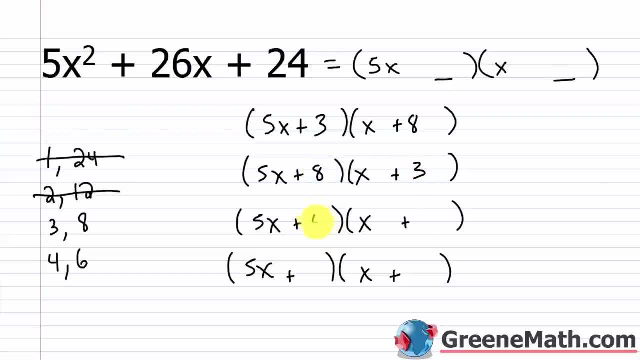 and 8.. And let's try 4 and 6 if we need to. Okay. so 5 times 8 is 40.. 3 times 1 is 3.. 43 is not going to work. 5 times 3 is 15.. And then 8 times 1 is 8.. 15 plus 8 is 23.. That's not going to work. So this: 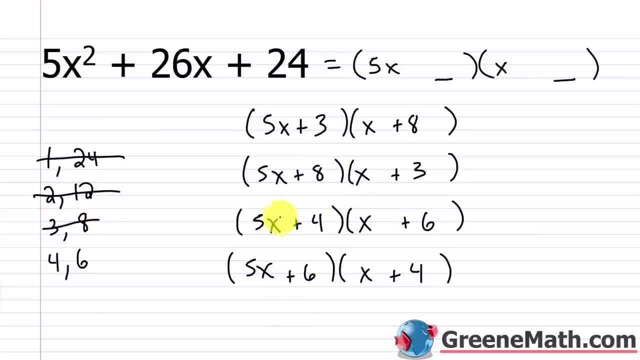 is eliminated. So now I'm down to the last possibility I have: 5 times 6. That's 30. And then 4 times 1 is 4.. That'd be 34.. And then, in this possibility, 5 times 4 is 20.. 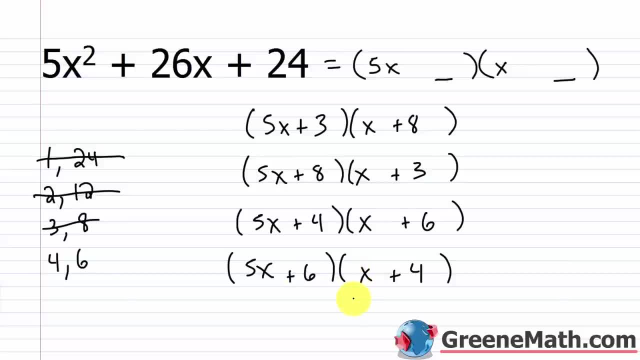 And then 6 times 1 is 6. That is 26.. Last one, So it's plus 6 and plus 4.. Let's erase all this. And again, that's the problem with trial and error. Sometimes you get it right away, Sometimes you have to go through all the. 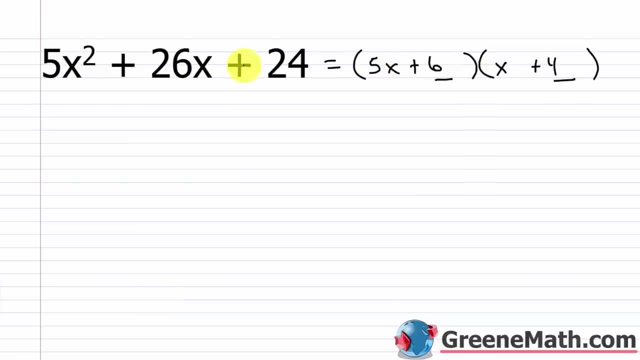 possibilities. You know you get it in the end. So 5x times x would be 5x squared, 5x times 4 would be 20x, 6 times x would be 6x. 20x plus 6x is 26x, And then 6 times 4 is 24.. I have 5 times 6. That's 30. And then 4 times 1 is 4. That would be 34. 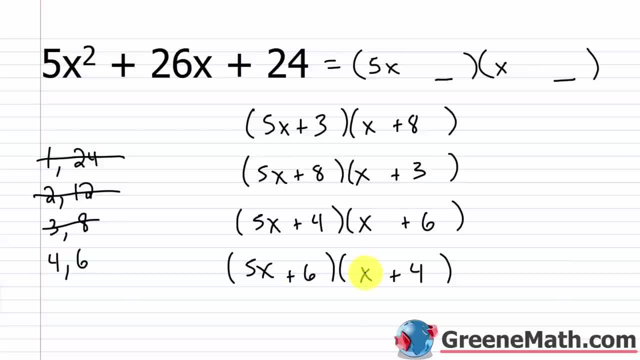 And then in this possibility, 5 times 4 is 20. And then 6 times 1 is 6. That is 26. 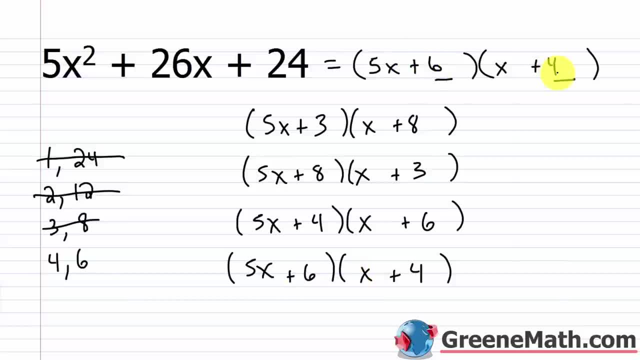 So it's the last one. So it's plus 6 and plus 4. 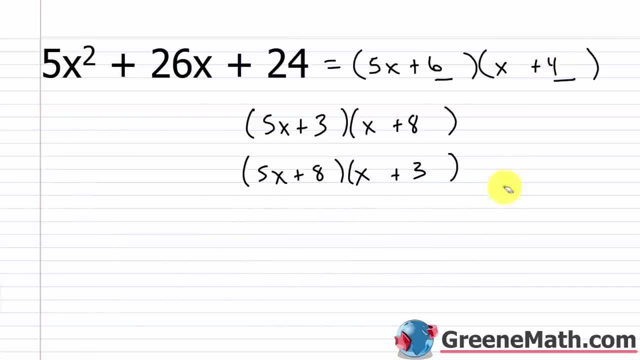 Let's erase all this. And again, that's the problem with trial and error. 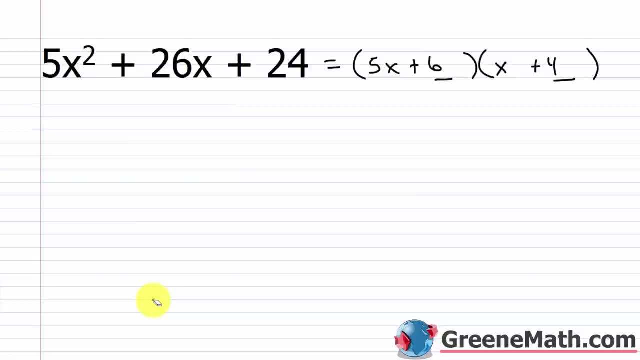 Sometimes you get it right away. Sometimes you have to go through all the possibilities. You know, you get it in the end. 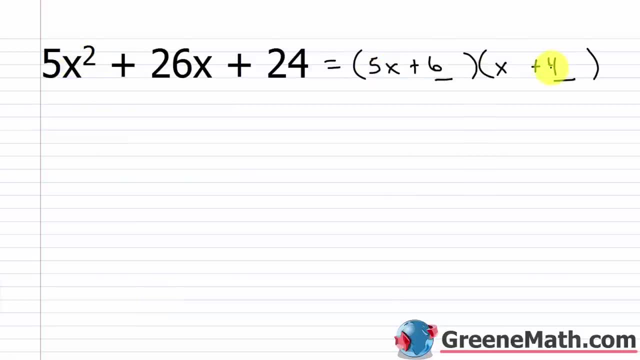 So 5x times x would be 5x squared. 5x times 4 would be 20x. 6 times x would be 6x. 20x plus 6x is 26x. And then 6 times 4 is 24. 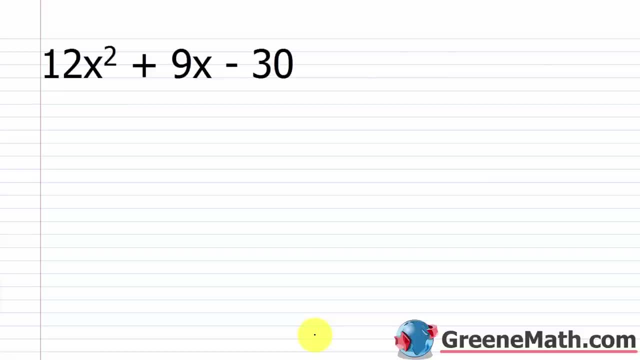 So what if we had 12x squared plus 9x minus 30? The first thing you notice is that this has a common factor of 3. So I could pull that 3 out. And I would have 4x squared. Plus. Plus 3x minus 10. So if I try to factor this as it is without pulling this out, that trick where I talked about you can't have a common factor in the binomial is not going to work. 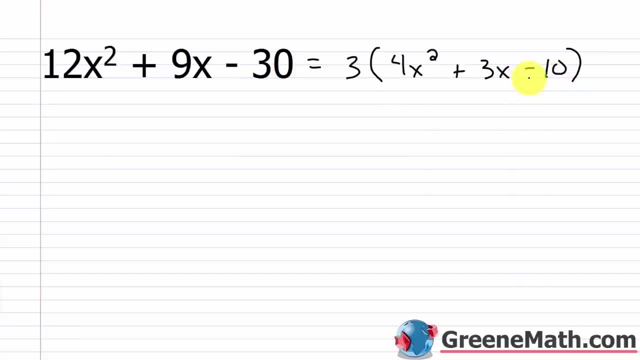 So that's why I do this to start. Make my life a lot easier. 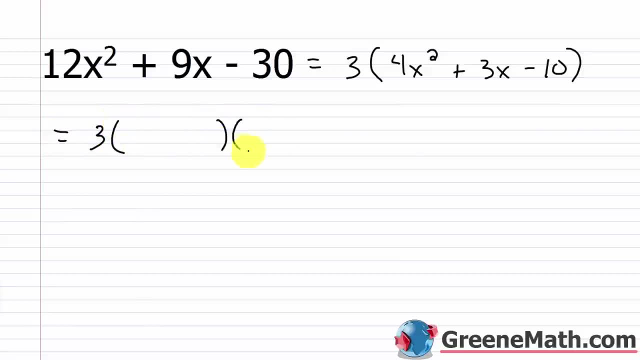 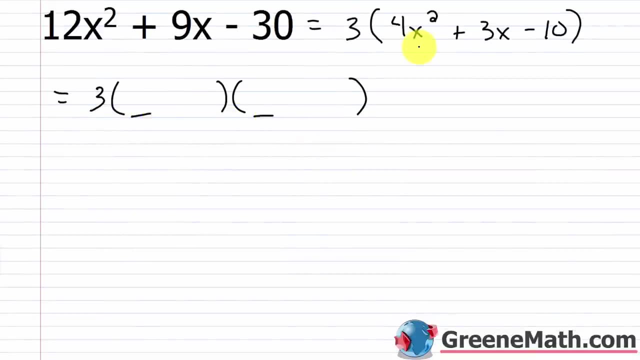 So again, if I set this up three times and have this scenario. So what would go here and here? For 4x squared, I could do a few different things. Let's start out by just looking at 2x and 2x. Right? So 2x times 2x would give me 4x squared. Then the possibilities for negative 10. 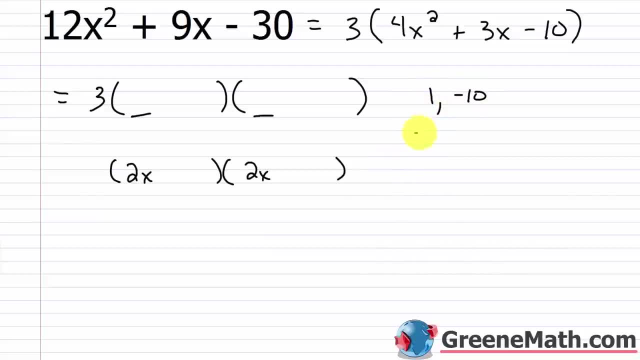 I've got 1 times negative 10. I've got negative 1 times positive 10. I've got negative 2 times 5. And I've got positive 2 times negative 5. So those are my possibilities. So let's run through these really quickly. And a lot of these we're going to be able to skip over. And I'll show you why. OK. 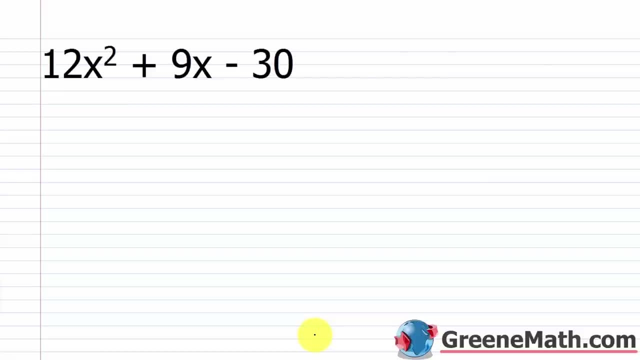 So what if we had 12x squared plus 9x minus 30?? The first thing you notice is that this has a common factor of 30.. So what if we had 12x squared plus 9x minus 30?? So what if we had 12x squared? 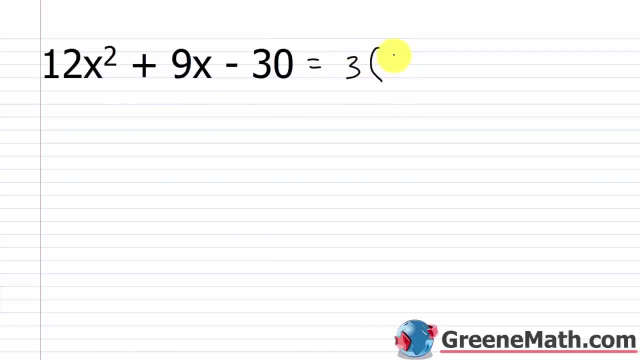 plus 9x minus 30?. So what if we had 12x squared plus 9x minus 30?? So I could pull that 3 out and I would have 4x squared plus 3x minus 10.. So if I try to factor this as it is, without pulling, 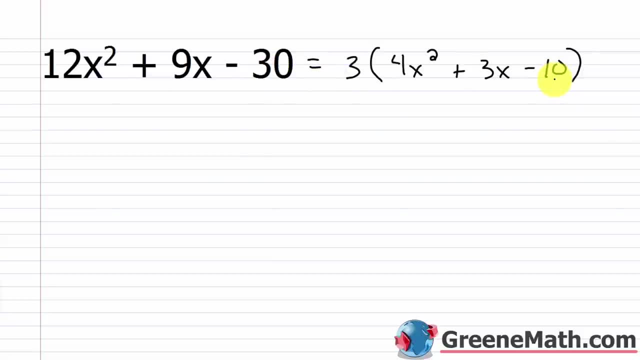 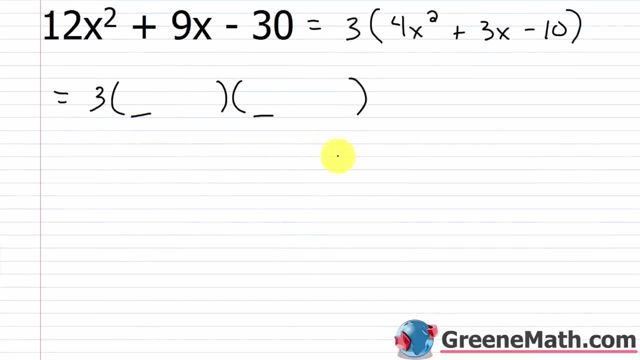 this out. that trick, where I talked about you can't have a common factor in the binomial- is not going to work. So that's why I do this, to start, Make my life a lot easier. So again, if I set this up three times and have this scenario, So what would go here and here? 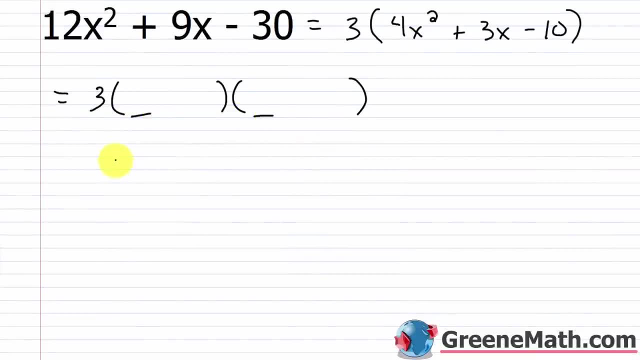 For 4x squared. I could do a few different things. Let's start out by just looking at 2x and 2x right. 2x times 2x would give me 4x squared. Then the possibilities for negative 10,. 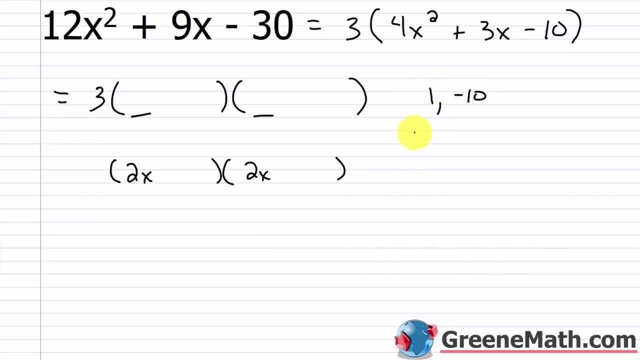 I've got 1 times negative 10.. I've got negative 1 times positive 10.. I've got negative 2 times 5. And I've got positive 2 times negative 5.. So those are my possibilities. So let's run through these really quickly And a lot of these we're going to be able to skip. 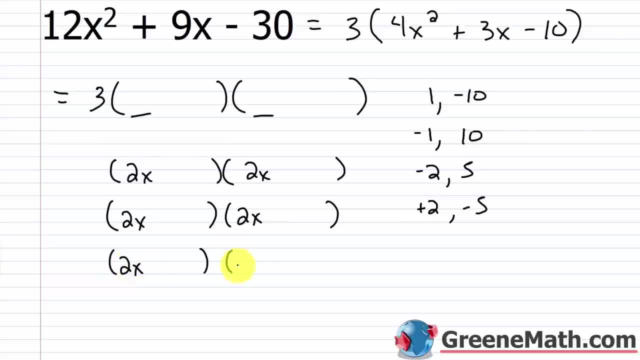 over. So let's run through these really quickly, And a lot of these we're going to be able to skip over, And I'll show you why. Okay, so if I want to use 1 and negative 10,, any way I do it, I'm going to have a common factor of. 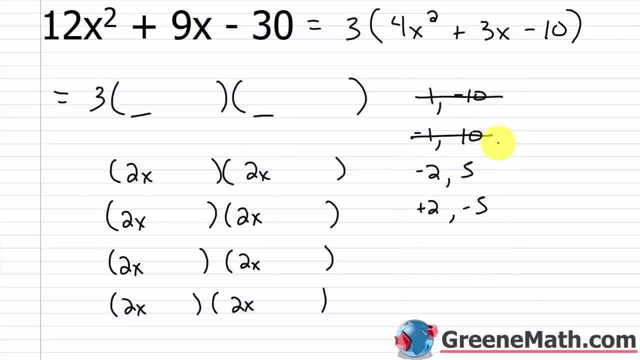 2. So I can eliminate that Again. same thing here: If I want to use negative 2 and 5, I'm going to have a common factor of 2. So that's eliminated And that's eliminated- either negative 2 or positive 2. Because I've got to put it on one of the sides. 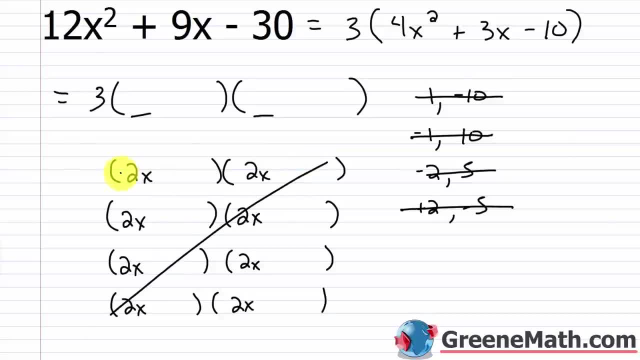 and I'd have a common factor of 2.. So I'm going to have a common factor of 2.. So I'm going to have a common factor of 2.. So I'm going to have a common factor of 2.. So this is eliminated right away. 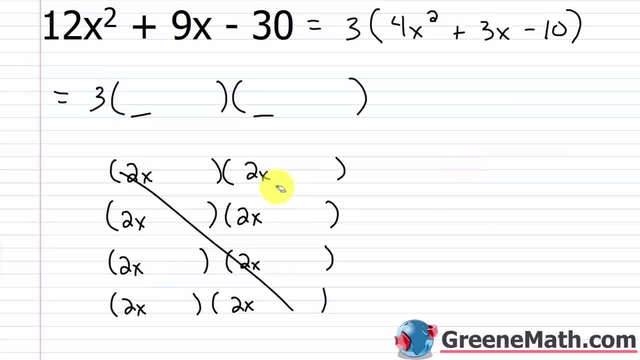 So I've got to go to a different one. I've got to go to 4x times x. Let's try that. So 4x, 4x, 4x, 4x, And then my x is over here. So then again the possibilities for negative 10,. 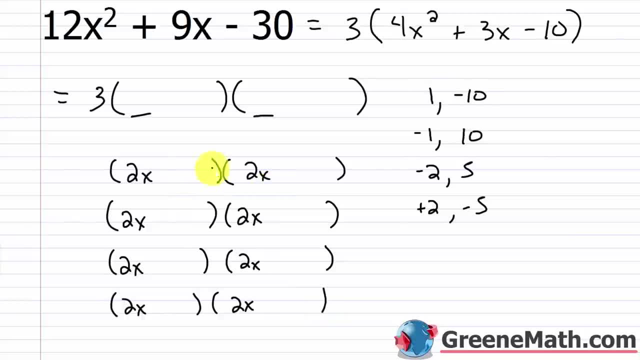 So if I want to use 1 and negative 10, any way I do it, I'm going to have a common factor of 2. So I can eliminate that. Again, same thing here. 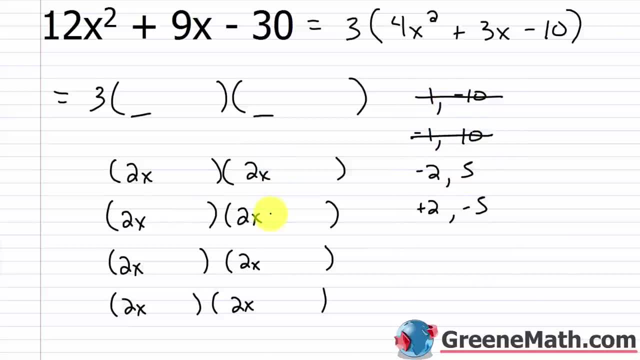 If I want to use negative 2 and 5, I'm going to have a common factor of 2. So that's eliminated. 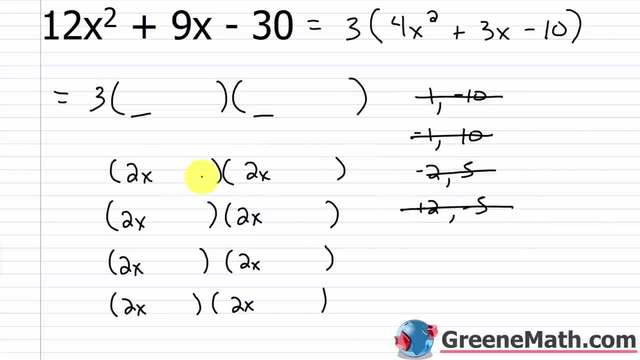 And that's eliminated, either negative 2 or positive 2. Because I've got to put it on one of the sides and I'd have a common factor. 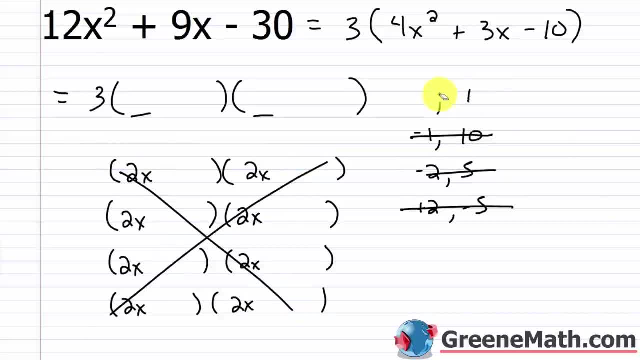 So this is eliminated right away. So I've got to go to a different one. I've got to go to. 4x times x. Let's try that. 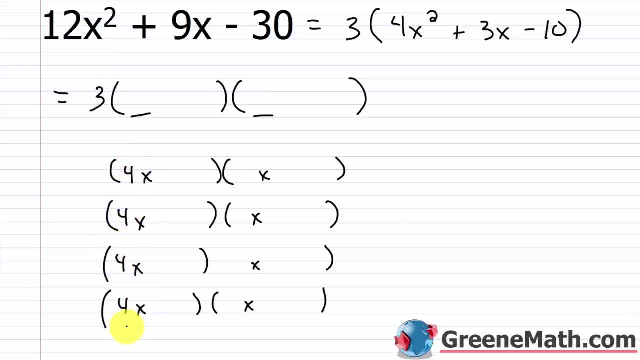 So 4x, 4x, 4x, 4x. And then my x is over here. So then again, the possibilities for negative 10, I've got negative 1 times 10. 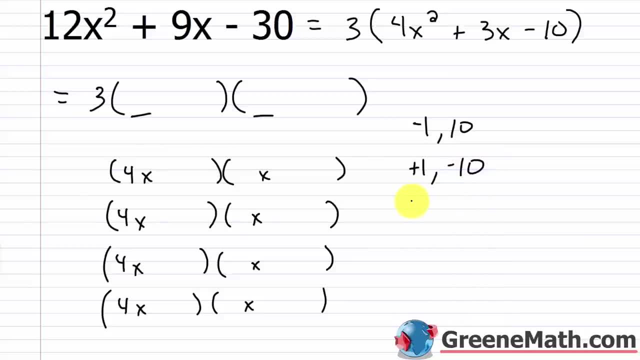 I've got positive 1 times negative 10. I've got 2 times negative 5. And I've got negative 2 times positive 5. 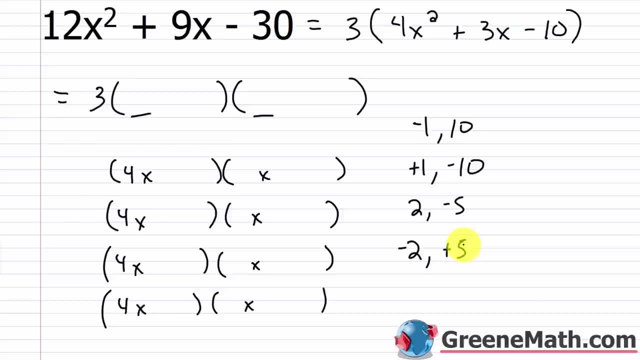 But again, because of the common factor thing, there's only so many arrangements I can use. So I can't do a 10 right here. 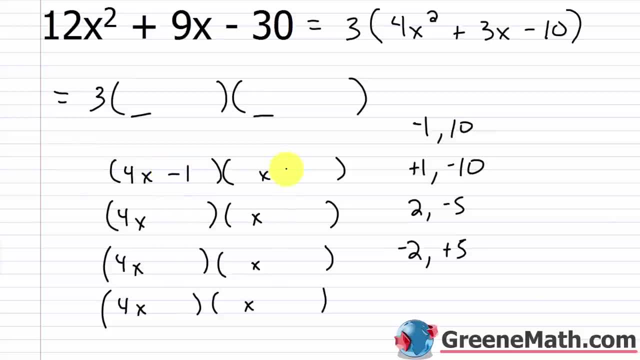 There'd be a common factor of 2. But I can do a negative 1 and I can do a positive 10. So 4x times 10 would be 40x. Negative 1 times x would be negative x. 40x minus x would be 39x. 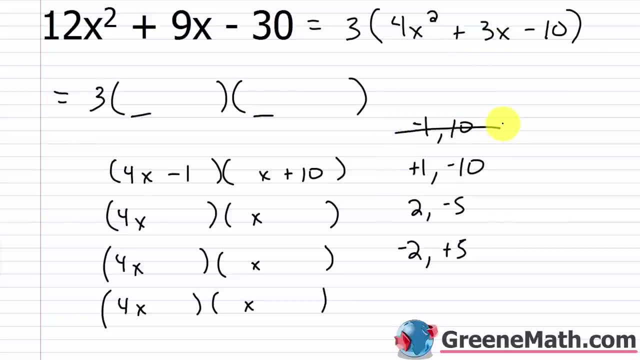 That's not going to get me 3x. I can get rid of that. 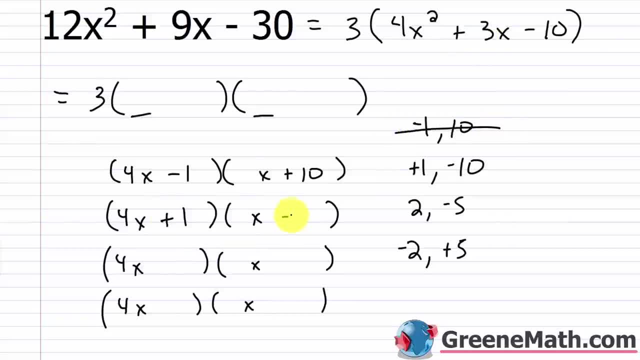 The next scenario, we could do plus 1 and negative 10. 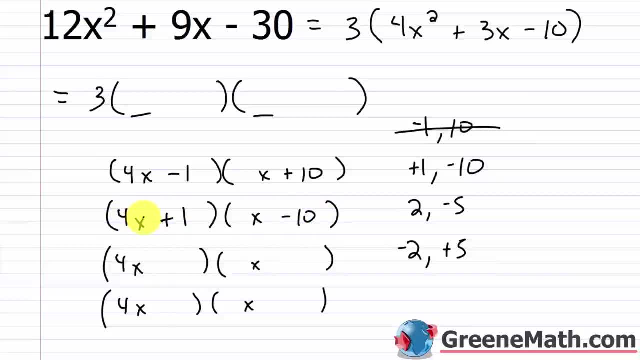 Again, I can't put a negative 10 over here because it would have a common factor of 2 with that 4. 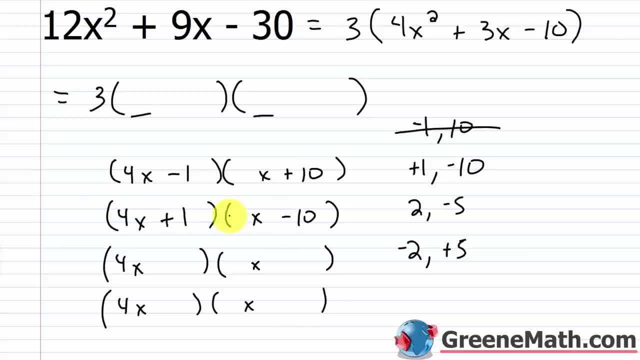 So 4x times negative 10 is negative 40x. 1 times x is x. That would be negative 39x. 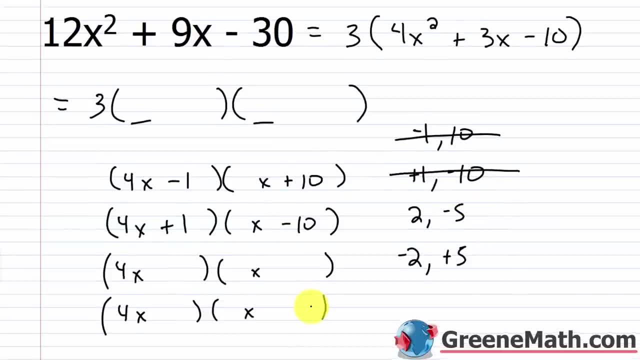 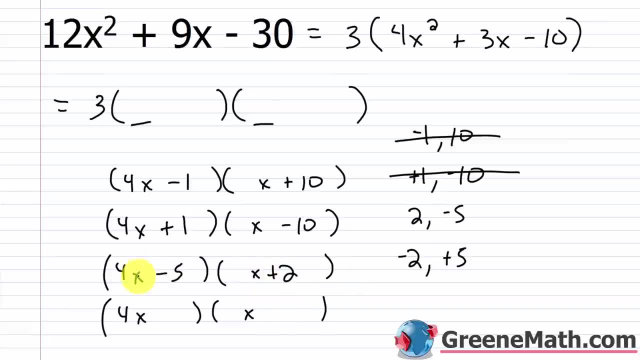 That's eliminated. So then the next one, we have 2 and negative 5. So it's got to be minus 5 and plus 2. Again, I can't put the 2 over here because it would have a common factor with the 4. And this right here doesn't have a common factor in it. It does in the original one, but we already pulled it out. So this should not have any common factor. 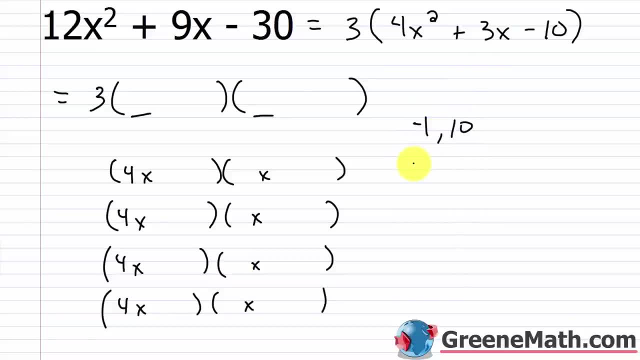 I've got negative 1 times 10.. I've got positive 1 times negative 10. I've got 2 times negative 5. And I've got negative 2 times positive 5. But again, because of the common factor thing, there's only so many arrangements I can use, So 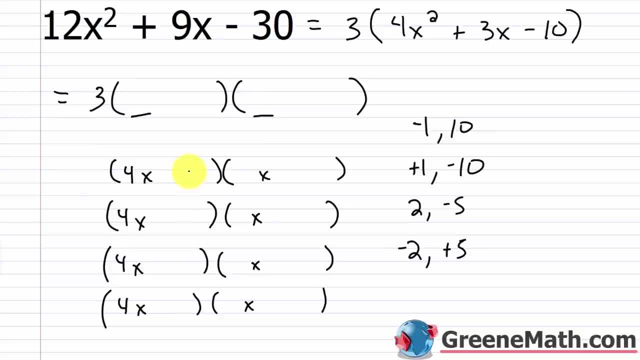 I can't do a 10 right here. There'd be a common factor of 2. But I can do a negative 1, and I can do a positive 10.. So 4x times 10 would be 40x Negative. 1 times x would be negative x. 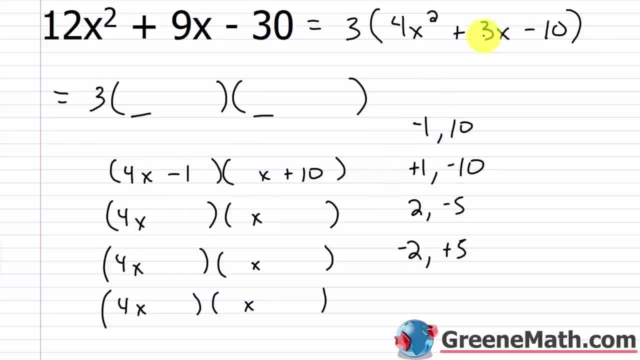 40x minus x would be 39x. That's not going to get me 3x. I can get rid of that. The next scenario we could do: plus 1 and negative 10.. Again, I can't put a negative 10 over here. 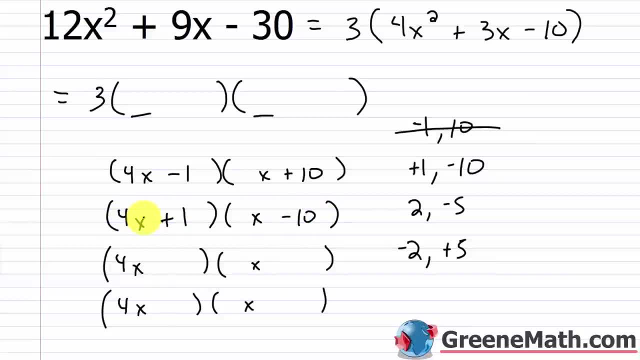 because it would have a common factor of 2 with that 4.. So 4x times negative, 10 is negative. 40x. 1 times x is x. That would be negative. 39x. That's eliminated. So then the next one. 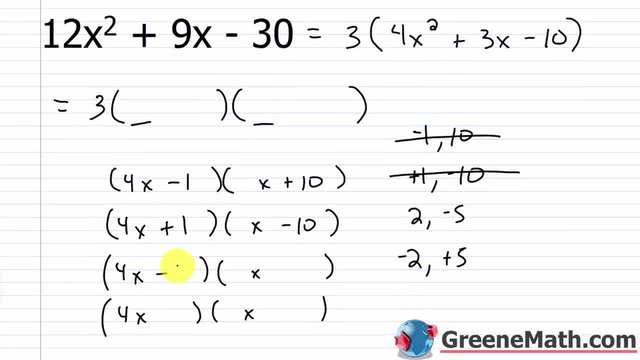 we have 2 and negative 5.. So it's got to be minus 5 and plus 2.. Again, I can't put the 2 over here because it would have a common factor with the 4.. So I can't put a negative 5 over here. I can't put. 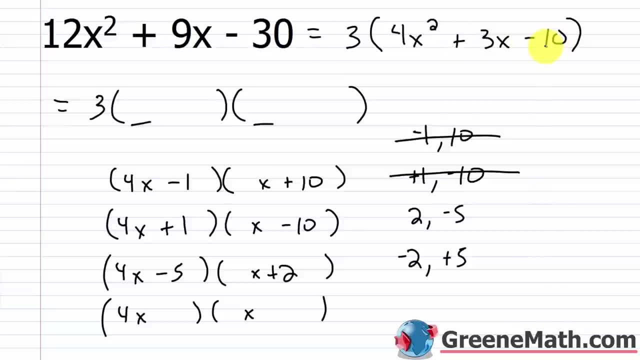 4. And this right here doesn't have a common factor in it. It does in the original one, but we already pulled it out, So this should not have any common factor when we consider what's inside the parentheses here and that's what we're factoring. Okay, So again, 4x times 2 would. 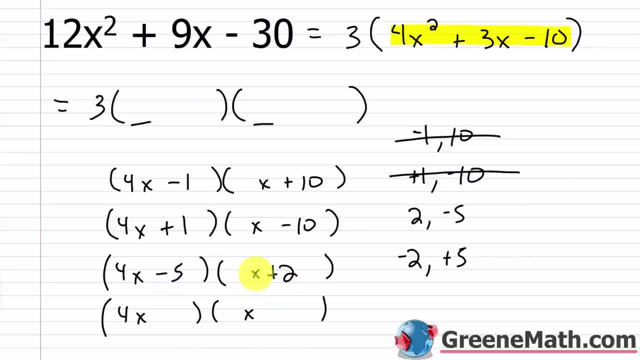 be 8x. Negative 5 times x would be negative 5x. So 8x minus 5x would be 3x. So this is what we're looking for right here. So let's erase everything and put 4x minus 5 times x. 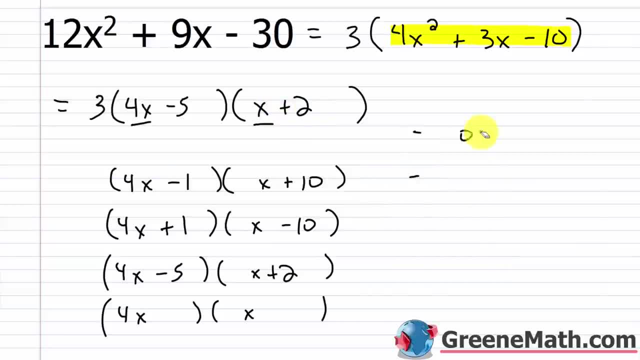 Plus 2.. So again, I know that a lot of you will use this method and you'll like it and that's fine. Again, I dislike it. I just think it's a little too tedious. I know there's tips and tricks. 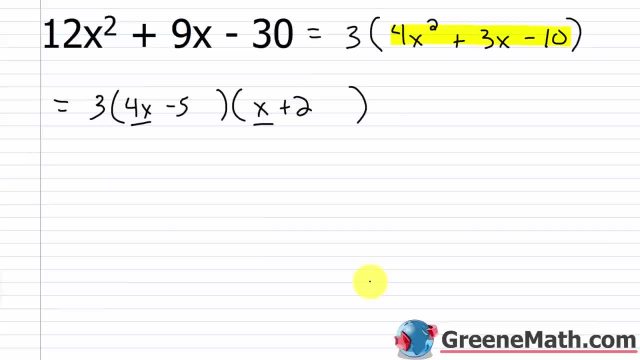 to speed it up even more, but I just don't care for it. So the end result here is 3 times the quantity 4x minus 5, and then times x plus 2.. And again, if you want to check it, 4x times x is 4x. 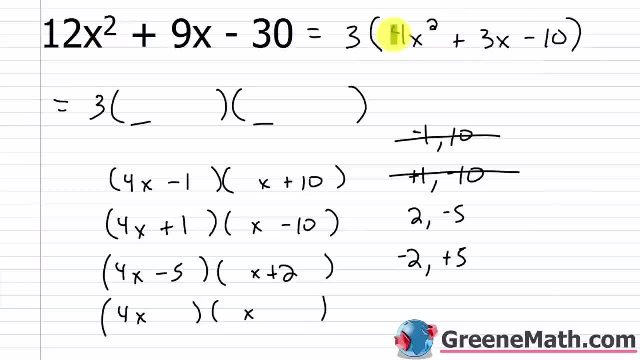 Common factor, when we consider what's inside the parentheses here, and that's what we're factoring. 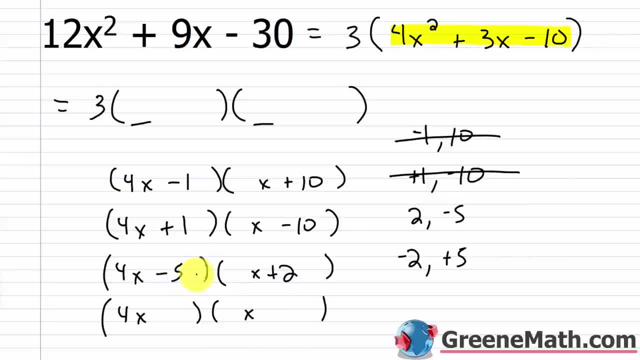 So again, 4x times 2 would be 8x. Negative 5 times x would be negative 5x. So 8x minus 5x would be 3x. So this is what we're looking for right here. 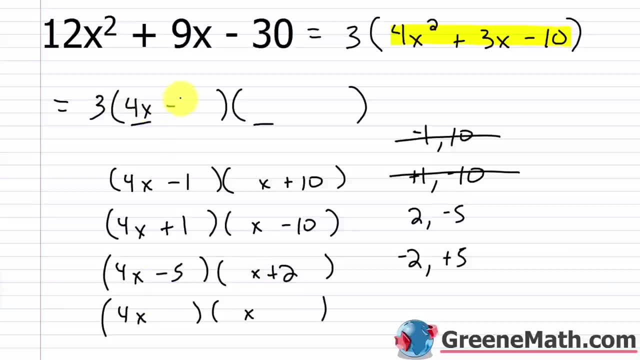 So let's erase everything and put 4x minus 5 times x plus 2. So again, I know that a lot of you will use this method, and you'll like it, and that's fine. 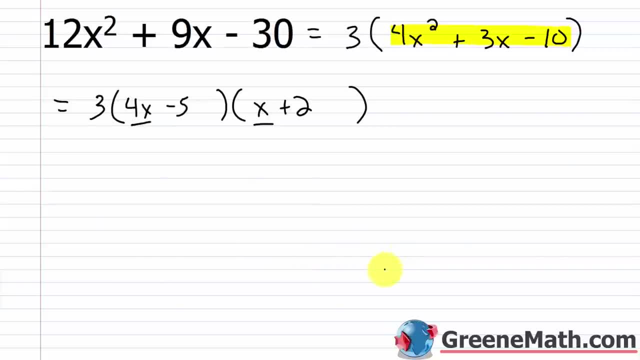 Again. I just like it. I just think it's a little too tedious. I know there's tips and tricks to speed it up even more, but I just don't care for it. 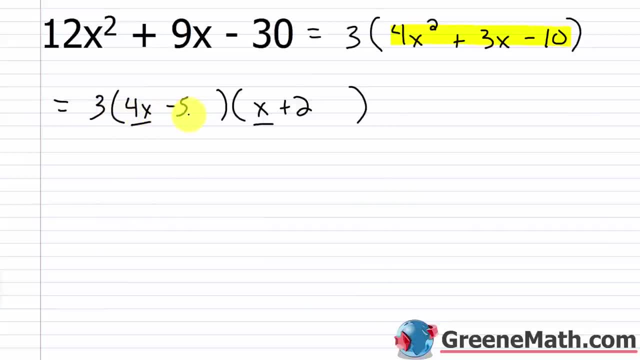 So the end result here is 3 times the quantity 4x minus 5, and then times x plus 2. And again, if you want to check it, 4x times x is 4x squared. The outer 4x times 2 is plus 8x. 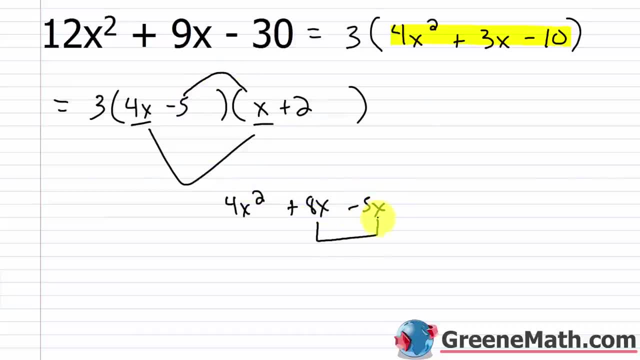 The inner negative 5 times x is minus 5x. So this would give me plus 3x. And then negative 5 times 2 is negative 10. So if we took 4x squared plus 3x minus 10, multiply it by 3, you get 12x squared plus 9x minus 30, which is what you started with. 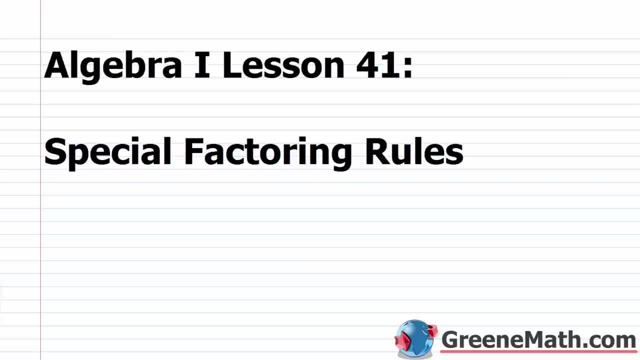 Hello, and welcome to Algebra 1, Lesson 41. In this video, we're going to learn about special factoring rules. 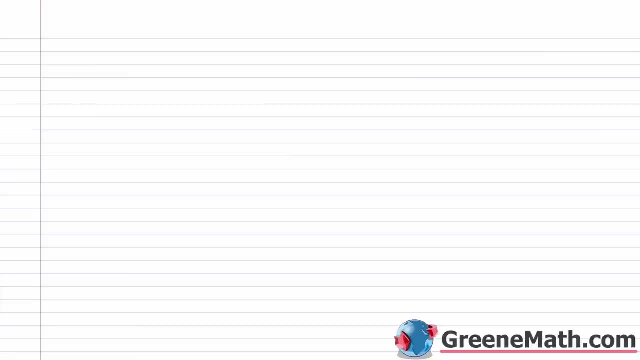 So back when we learned how to multiply polynomials, we did a lesson on special products. And that lesson was meant to greatly increase your speed when you had to find certain polynomial products that occurred very often. So for example, one of the ones we looked at, we looked at x plus y, that quantity squared. And you know it's the first term squared plus 2 times the first term times the second term, so 2xy, and then plus the final term squared, so y squared. 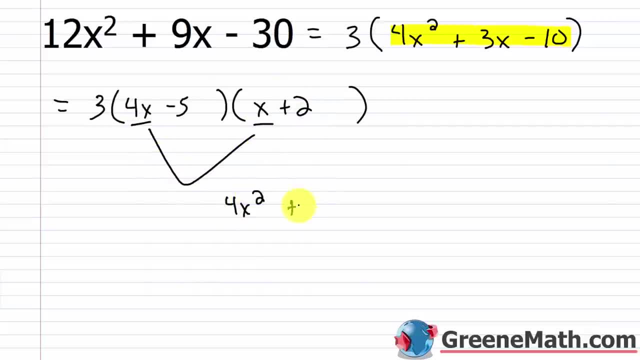 squared, The outer 4x times 2 is plus 8x, The inner negative 5 times x minus 5x. So this would give me plus 3x And then negative 5 times 2 is negative 10.. So if we took 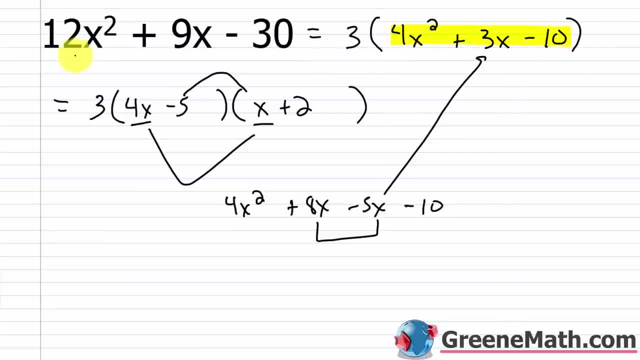 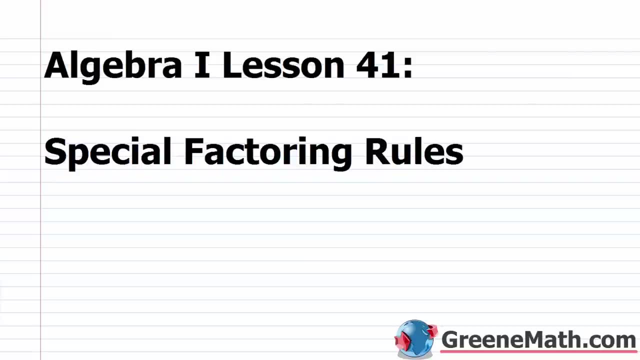 4x squared plus 3x minus 10, multiply it by 3, you get 12x squared plus 9x minus 30, which is what you started with. Hello and welcome to Algebra 1, Lesson 41.. In this video, we're going to learn: 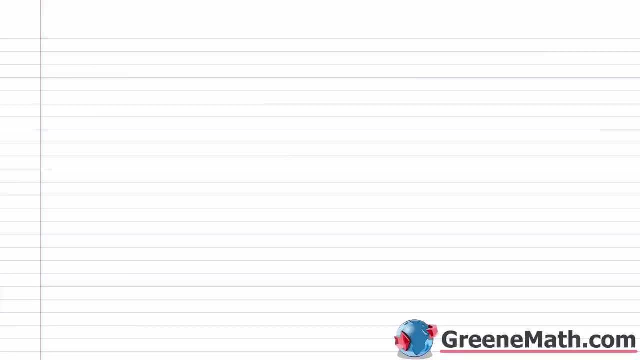 about special factoring rules. So back when we learned how to multiply polynomials, we did a lesson on special products, And that lesson was meant to greatly increase your speed when you had to find certain polynomial products that occurred very often. So, for example, one of the ones we looked at, we looked at x plus. 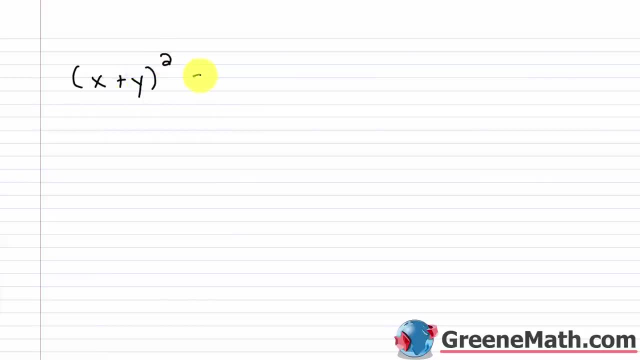 y, that quantity squared- And you know it's the first term- squared, plus two times the first term, times the second term, so 2xy, and then plus the final term squared, so y squared. So without using FOIL I'm able to multiply that instantly And you could look at an example. that's: 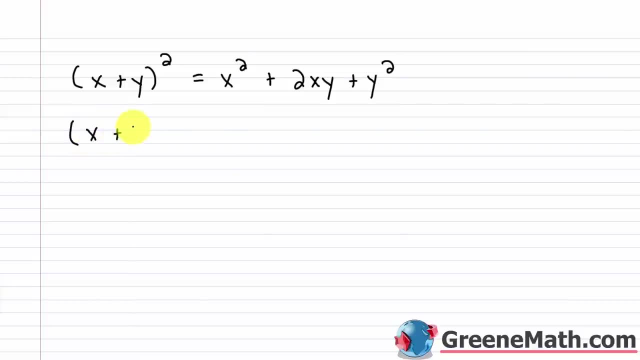 not generic. You could do something like, let's say x plus 5,, that quantity squared, So that would be x squared plus 2 times x times 5, so that's 10x, And then plus that last term, which is 5. 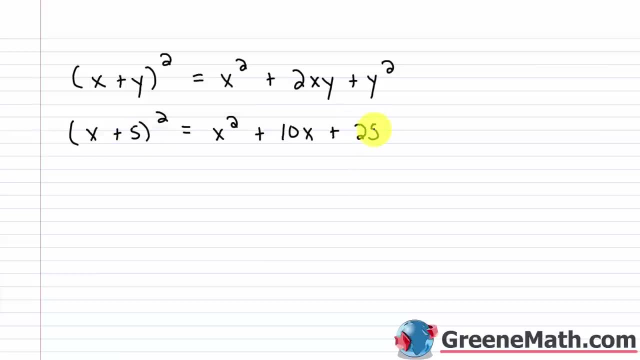 squared, that's 25.. So I'm able to use that formula to very quickly get the answer. Now we saw this on a few different things. We also looked at kind of this with a minus sign: So x minus y, that quantity squared, And the only thing that changed here was the sign. So it was x squared. 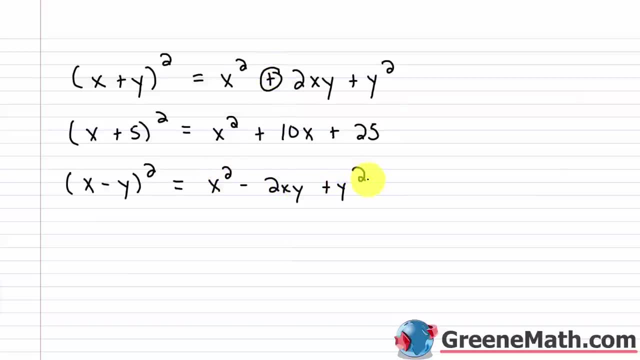 minus 2xy plus y squared. So as another example with just numbers, let's say we made this a little bit more complex. We said: this is 4x minus 5, that quantity squared. Well, the first term here, 4 and the x would be squared. So 4 and the x, that's all squared Then, minus the first term. 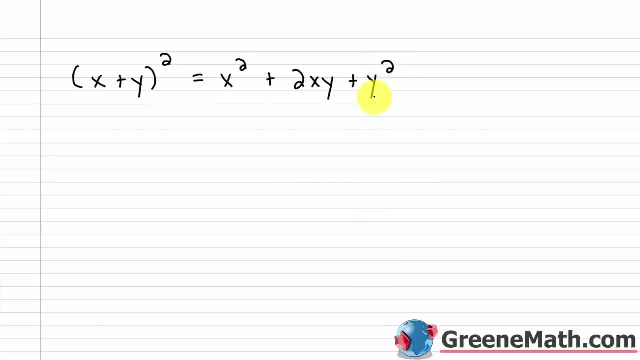 So without using FOIL, I'm able to multiply that instantly. And you can look at an example that's not generic. You could do something like this. Something like, let's say, x plus 5, that quantity squared. So that would be x squared plus 2 times x times 5, so that's 10x. And then plus that last term, which is 5 squared, that's 25. So I'm able to use that formula to very quickly get the answer. Now, we saw this on a few different things. 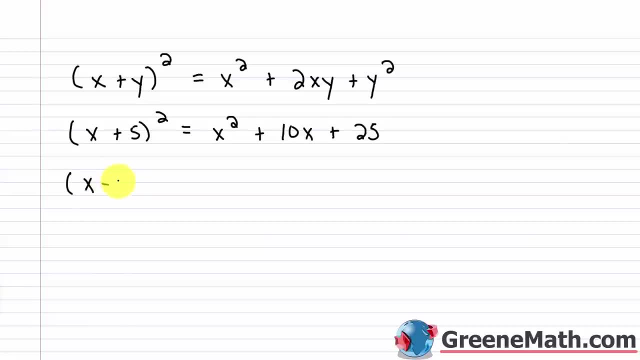 We also looked at kind of this with a minus sign, so x minus, 1. 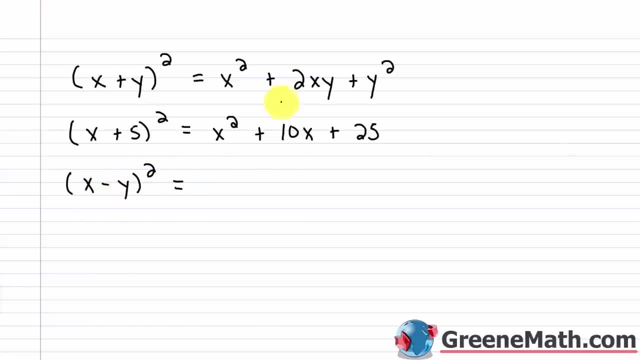 y that quantity squared and the only thing that changed here was the sign so it was x squared minus 2x y plus y squared so as another example with just 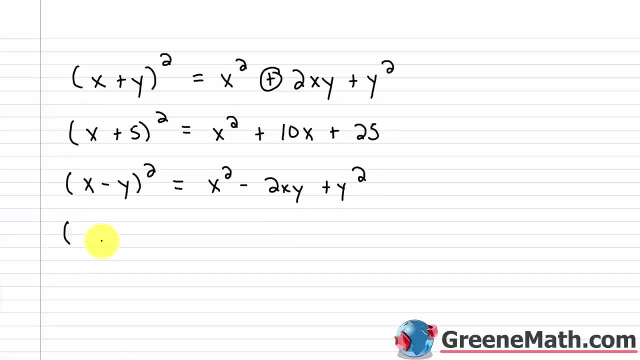 numbers let's say we made this a little bit more complex we said this is 4x minus 5 that quantity squared well the first term here the 4 and the X would be 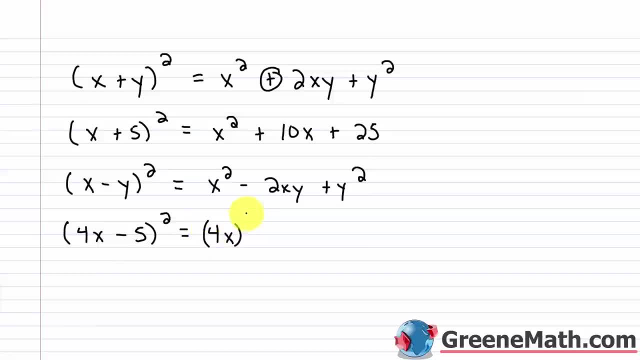 squared so 4 and the X that's all squared then minus the first term times the second term times 2 so 2 times 4 is 8 8 times 5 is 40 then times X so minus 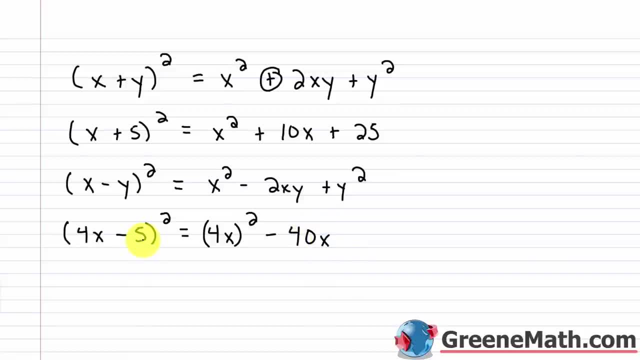 40 X and then we have our final term which is 5 that would be squared so plus 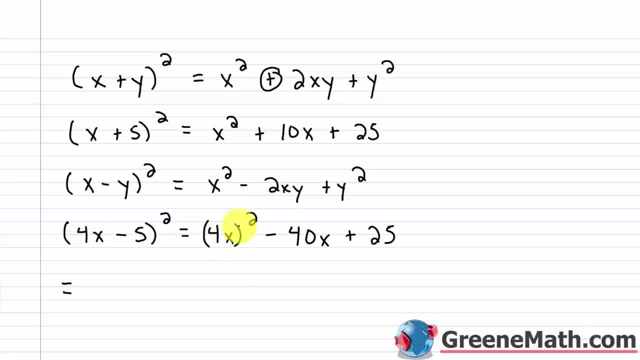 25 so to simplify this 4 squared is 16 and X squared is just x squared so this would be 16x squared 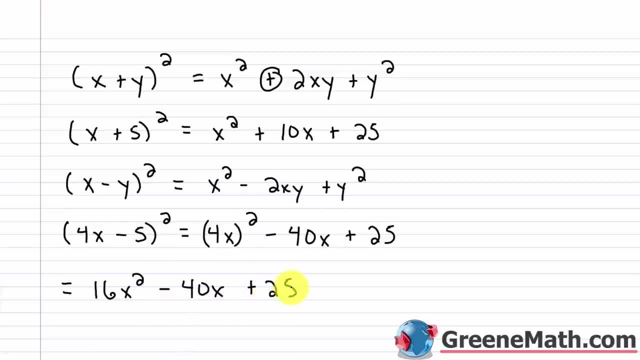 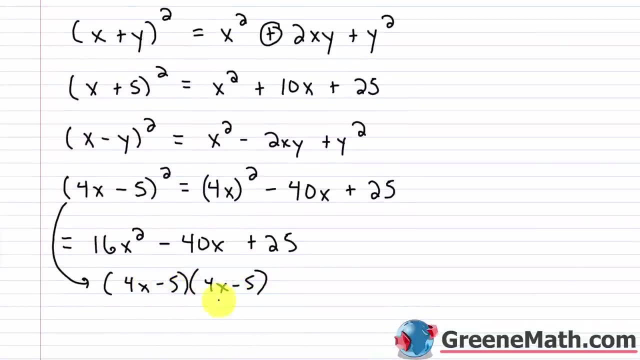 minus 40x plus 25. So a much quicker way to do that versus going, okay, well, this is 4x minus 5 times 4x minus 5. You know, first times first is 16x squared and outer is minus 20x 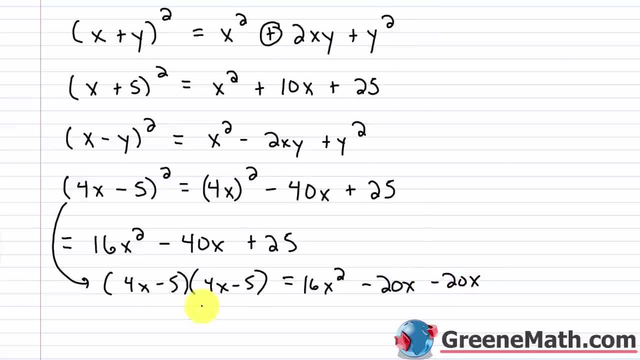 and inner is minus 20x and last is plus 25. You know, combine like terms here and get this over here. So let's kind of reverse this process. We already know how to do the multiplication part. 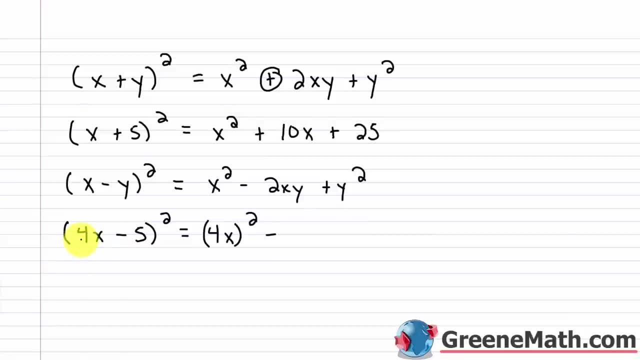 times the second term, times 2.. So 2 times 4 is 8.. 8 times 5 is 40. Then times x, so minus 40x, And then we have our final term, which is 5.. That would be squared, so plus 25.. So to simplify this: 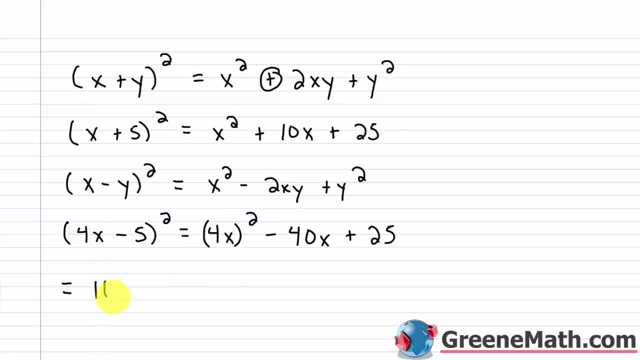 4 squared is 16, and x squared is just x squared. So this would be 16x squared Minus 40x plus 25.. So a much quicker way to do that versus going okay. well, this is 4x minus 5. 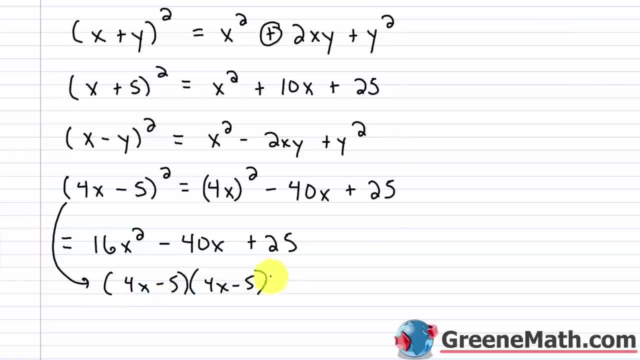 times 4x minus 5.. First times: first is 16x squared And outer is minus 20x And inner is minus 20x And last is plus 25.. Combine like terms here and get this over here. So let's kind of. 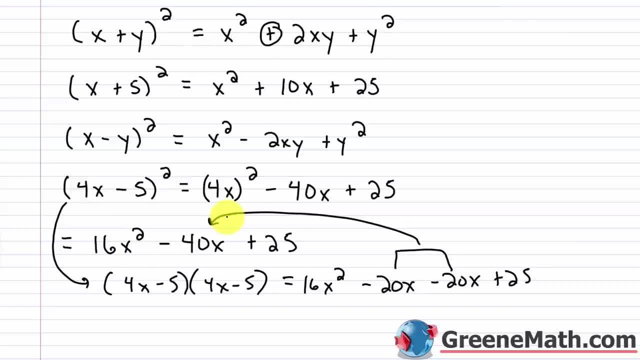 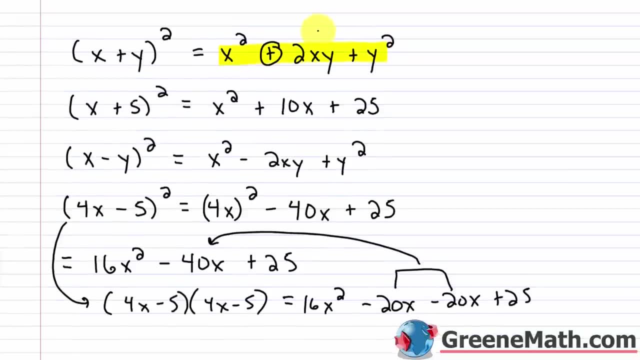 reverse this process. We already know how to do the multiplication part. We've already gone through that lesson, So now what we're going to do is learn how to take something in this format and put it in this format. We're going to factor it, So we're going to start out. 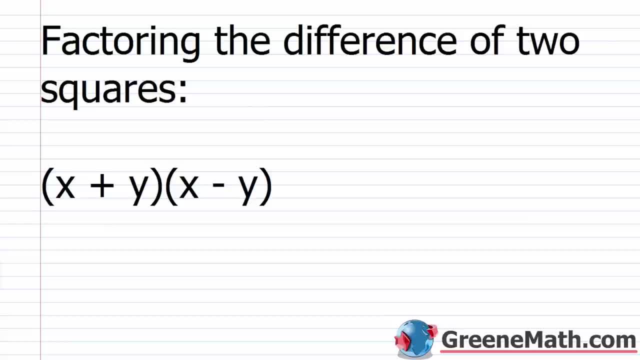 by factoring the difference of two squares. So remember when we went to our lesson on special products, we had the quantity x plus y times the quantity x minus y. So it's the same thing and here and the same thing here and here. So in other words, the first position of each is x. The 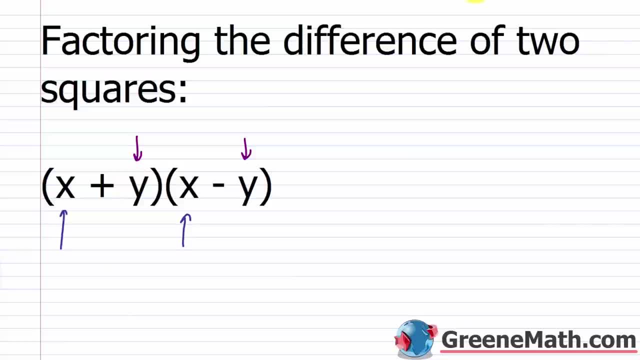 second position of each is y. What is different is going to be your signs right, The plus and the minus. So this turns out to be the x, what's in the first position of each squared, minus the y, what's in the second position of each squared. Remember the middle. two terms are going to drop. 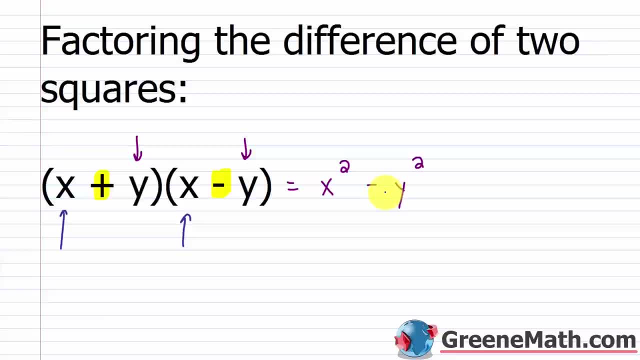 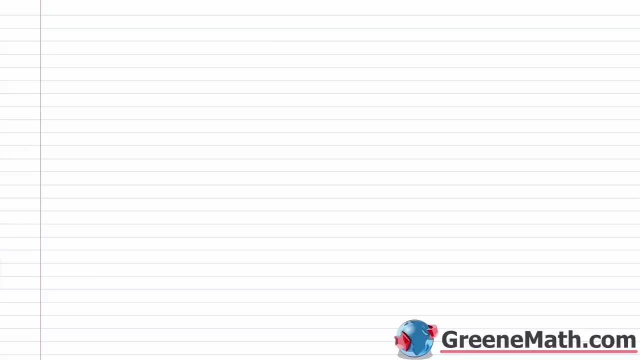 out right, Because the difference of the signs makes them cancel. So you get x squared minus y squared. So in this lesson we're going to go from this format to this format. So the first question you would ask is: how can we identify a binomial as the difference of two squares? 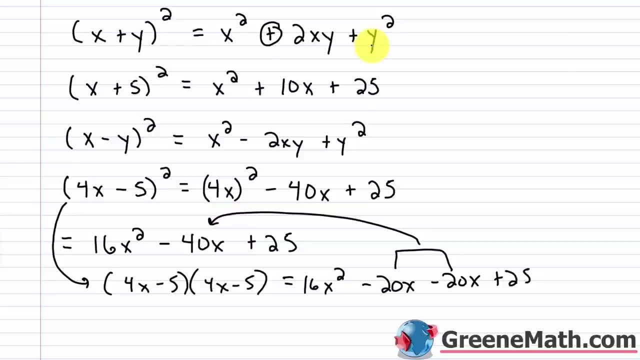 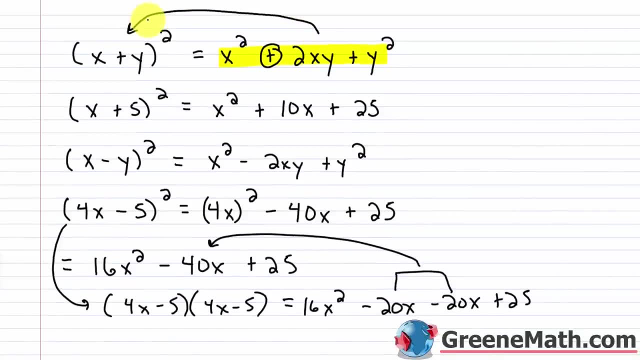 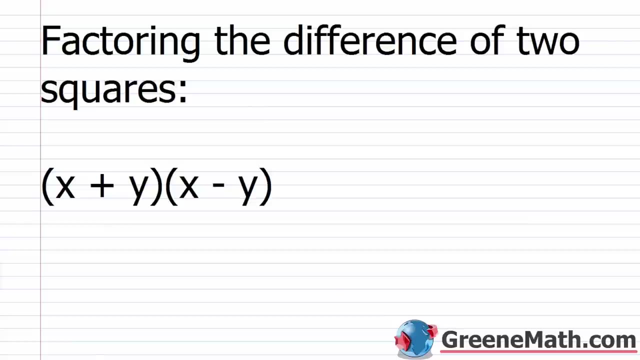 We've already gone through that lesson. So now what we're going to do is learn how to take something in this format and put it in this format. We're going to factor it. So we're going to start out by factoring the difference of two squares. So remember, when we went to our lesson on special products, we had the quantity x plus y times the quantity x minus y. So it's the same thing here and here and the same thing here and here. So in other words, the first position of each is x, the second position of each is y. What is different is going to be your sides, right? The plus and the minus. So this turns out to be the x, what's in the first position of each squared, minus the y, what's in the second position of each squared. Remember, the middle two terms are going to drop out, right? Because the difference of the signs makes them cancel. So you get x squared minus y squared. 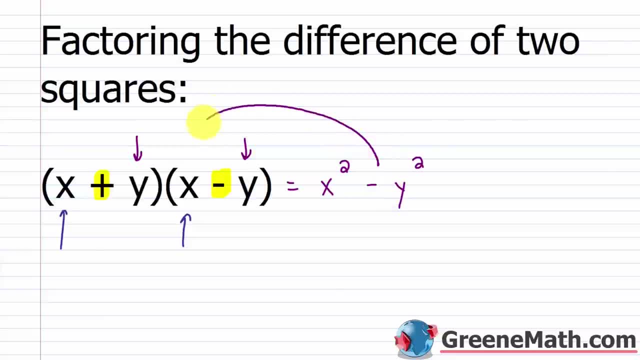 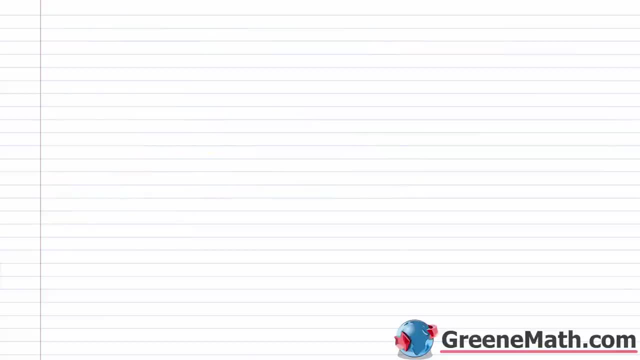 So in this lesson, we're going to go from this format to this format. So the first question you would ask is how can we identify a binomial as the difference of two squares? Well, the first 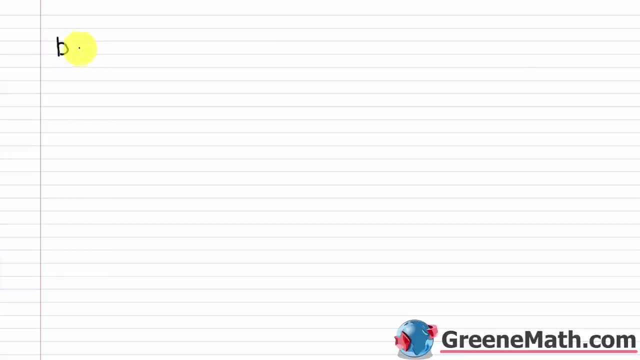 thing is that both terms, both terms must be squares. 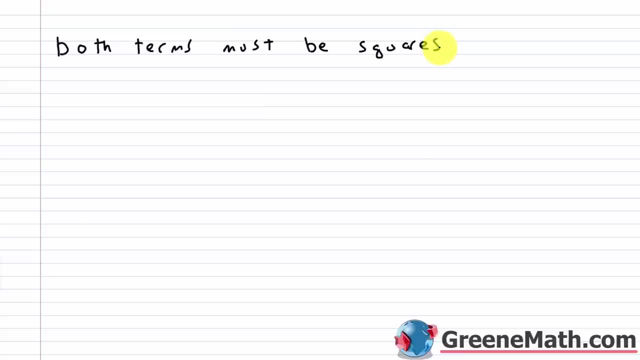 And what do I mean when I say both terms must be squares? Well, when we square something, we multiply it by itself. So in other words, if I have two squared, I know that's two times two or four. We know that at this point. But if I looked at the number four, I've got to be able to identify that that was created or can be created from two times two. And I know there's other ways to get four. It could be one times four. It could be, you know, negative two times negative two. 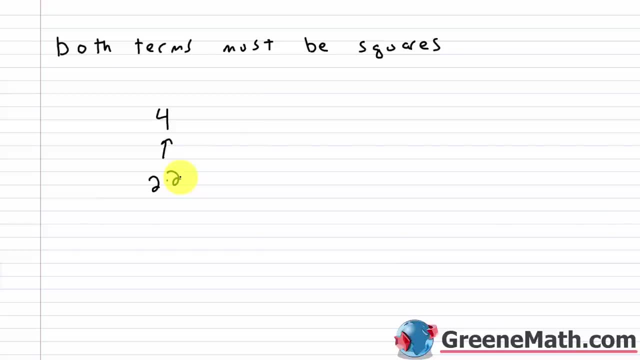 All these different variations. But you're looking for numbers or variables that can be created 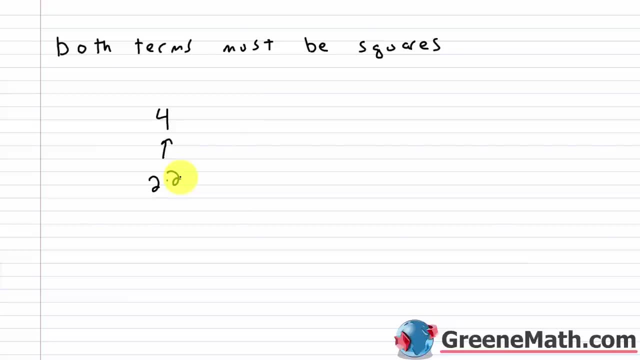 from some number or some variable multiplied by itself. So for example, if I have the number nine, that's three times three. And again, it could be other things. It could be nine times one. It could be negative three times negative three. But, you know, let's keep things positive and keep 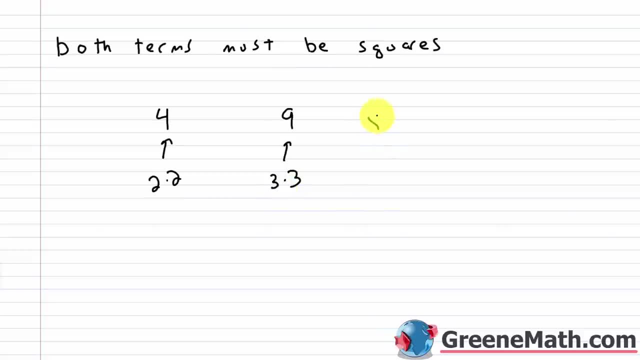 everything very simple. If I had a variable like x squared, well, this is x times x. Or I could make this much more complicated. 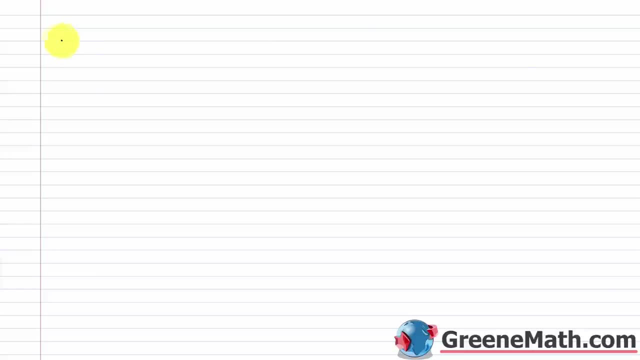 Well, the first thing is that both terms, both terms must be squares. And what do I mean when I say both terms must be squares? Well, when we square something, we multiply it by itself. So, in other words, if I have two, 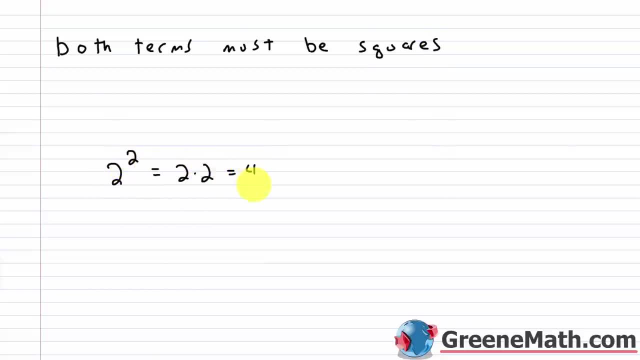 squared. I know that's two times two or four. We know that at this point. But if I looked at the number four, I've got to be able to identify that that was created or can be created from two times two. And I know there's other ways to get four. It could be one times four, It could be, you know. 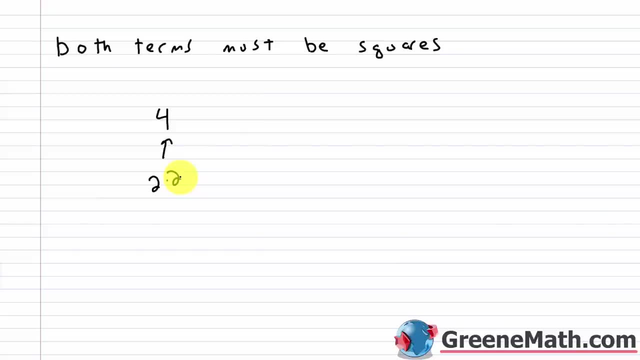 negative two times negative two. all these different variations. But you're looking for numbers or variables that can be created from some number or some variable multiplied by itself. So, for example, if I have the number nine, that's three times three, And again it could be other. 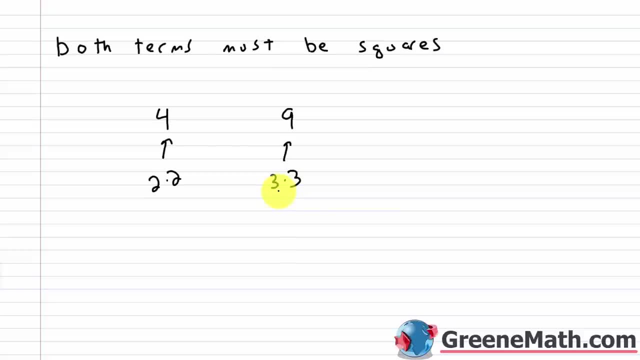 things. It could be nine times one. It could be negative three times negative three. But you know, let's keep things positive and keep everything very simple. If I had a variable like x squared well, this is x times x. Or I could make this much more complicated If I have a variable. 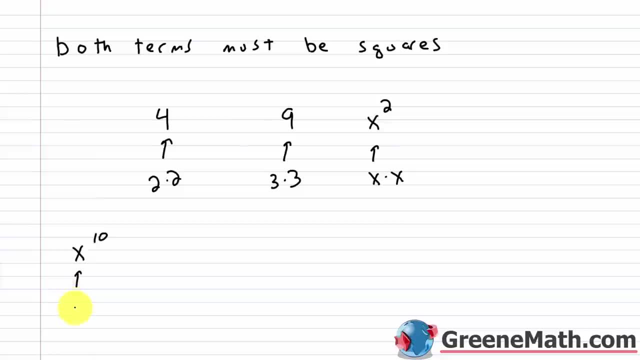 like, let's say x to the 10th power. Well, this could be x to the fifth power. That's squared right, Because if we keep the base the same and we multiply exponents, this would be x to the power of five times two, which is 10.. So 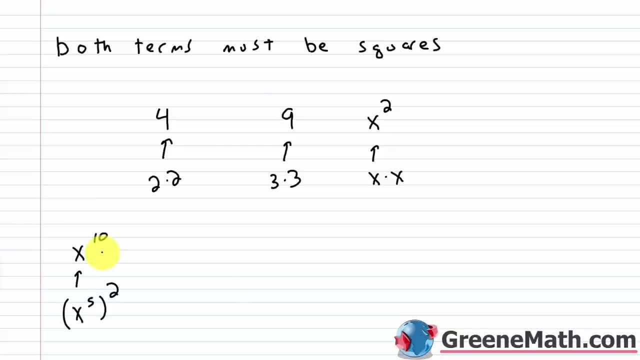 x to the 10th power is really x to the fifth power squared. Or if I wanted to do something like a number and a variable, let's say I did something like 25. y to the eighth power- Well, 25, I know, is five times five- And y to the eighth power. I could write as: 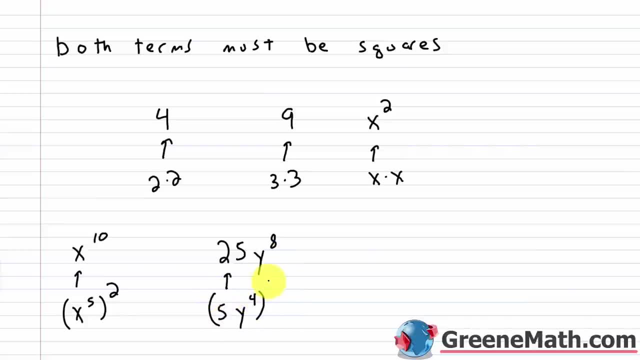 y to the fourth power. So if I squared this whole thing here, this would be five times five or 25.. And y to the fourth power squared. remember, keep y the same. multiply the exponents four times two is eight. So five y to the fourth power squared would give me 25 y to the eighth. 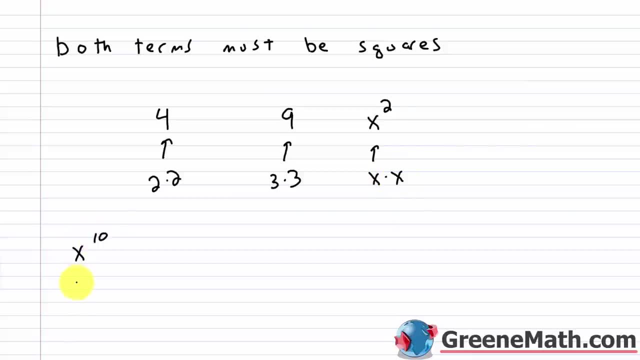 If I have a variable like, let's say, x to the 10th power. Well, this could be x to the fifth power. That's squared, right? Because if we keep the base the same and we multiply exponents, this would be x to the power of five times two, which is 10. So x to the 10th power is really x 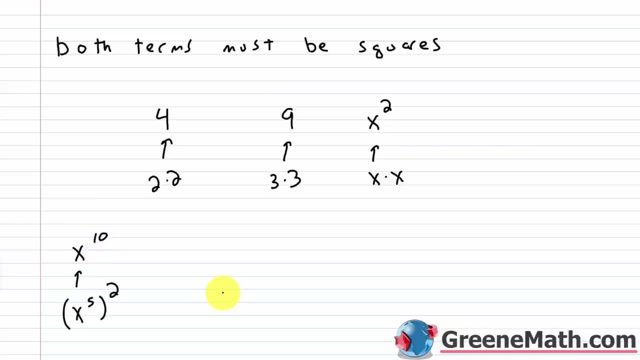 to the fifth power squared. Or if I wanted to do something like a number and a variable, let's say I did something like 25y to the eighth power. Well, 25, I know, 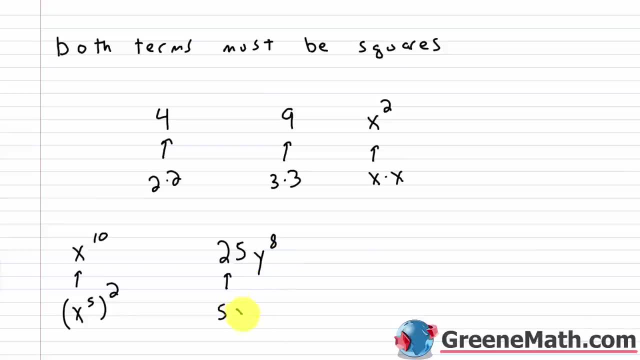 it's five times five. And y to the eighth power, I could write as y to the fourth power. So if I squared this whole thing here, this would be five times five or 25. And y to the fourth power squared, remember, keep y the same, multiply the exponents, four times two is eight. So five y to 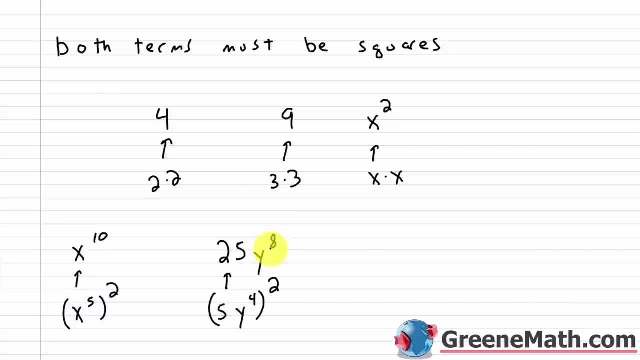 the fourth power squared would give me 25y to the eighth power. So this is what you're looking for 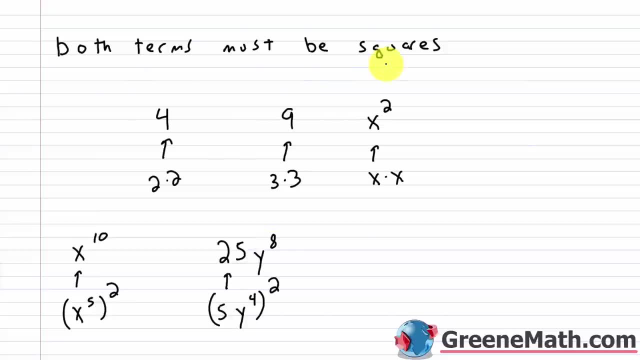 when you're looking for the difference of two squares. So both terms must be squares. Now, the other thing is that the second term is going to be negative. So your second term is negative. Now, I say that, and let me put a little notation next to it. This can be 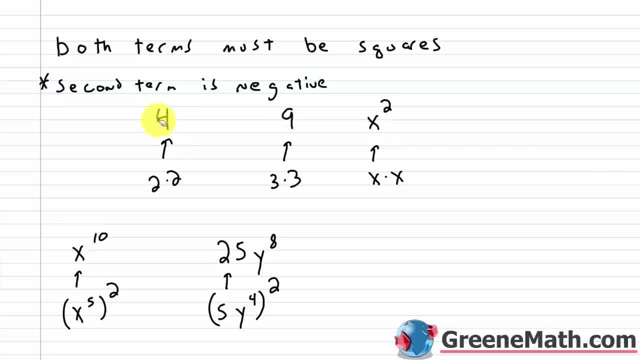 changed around. Because remember, if we have something with addition and subtraction, we can flip things around into a different order. So your teacher might try to trip you up. 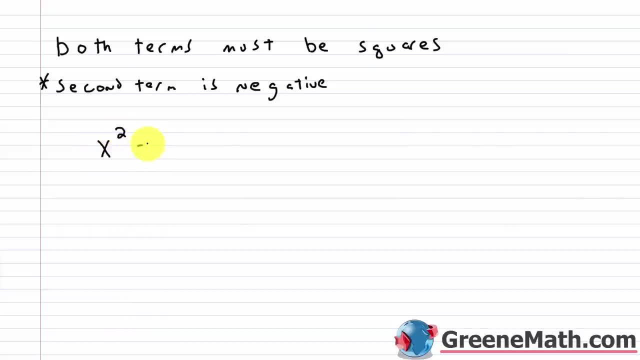 Let's say you saw something like this. And you're like, oh, my God, I'm going to do this. Something like x squared minus y squared. You know, this is the difference of two squares. 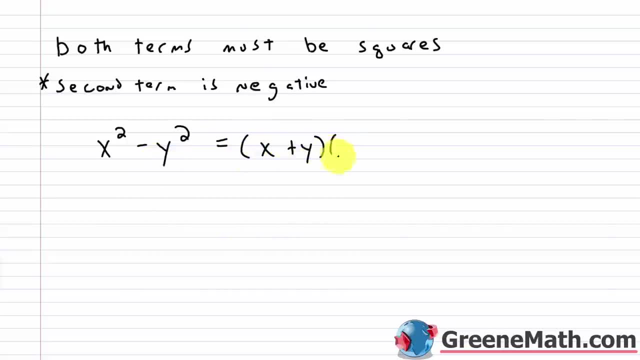 We already seen that this can factor into x plus y times x minus y. So another way you might see this presented, your teacher might try to trip you up. And she might say, okay, well, you have negative y squared plus x squared. Well, it's not that the second term is negative now. But remember, I could reorder these, I could change this into this, and it would still factor the same, 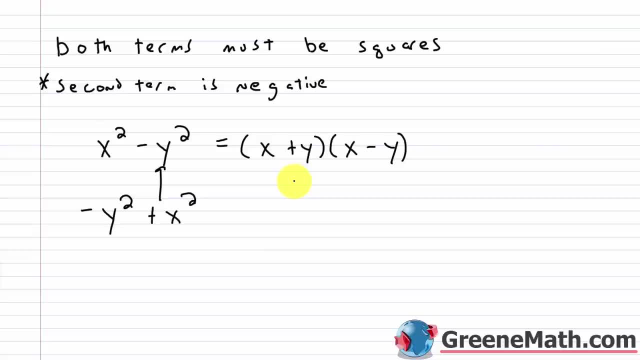 way. So just pay close attention that you want one of the terms to be positive, and one of the terms to be negative. So those are the two conditions. Alright, so let's start out with an 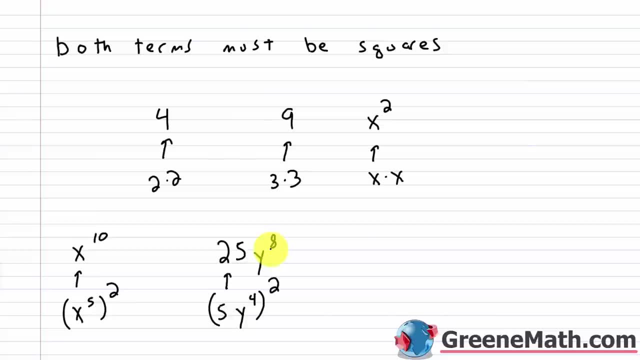 power. So this is what you're looking for when you're looking for the difference of two squares, So both terms must be squares. Now the other thing is that the second term is going to be negative. So your second term is negative. Now I say that, and let me put a little notation next. 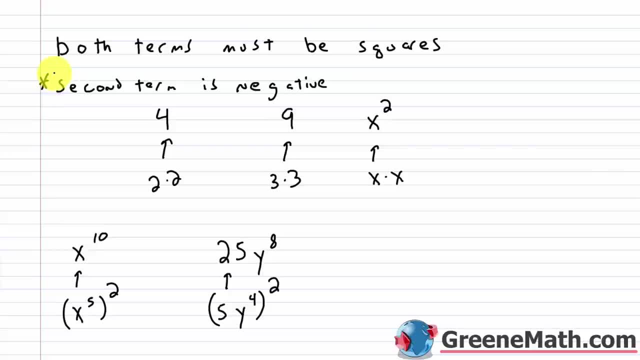 to it. This can be changed around Because, remember, if we have something with addition and subtraction, we can flip things around into a different order. So your teacher might try to trip you up. Let's say you saw something like x squared minus y squared. 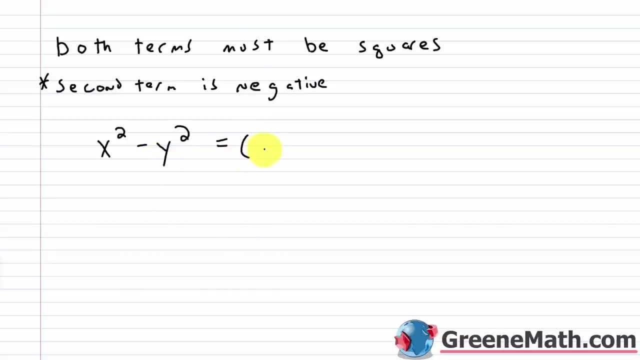 You know this is the difference of two squares. We've already seen that this can factor into x plus y times, x minus y. So another way you might see this presented. your teacher might try to trip you up And she might say: OK, well, you have negative y squared plus x squared. Well, it's not. 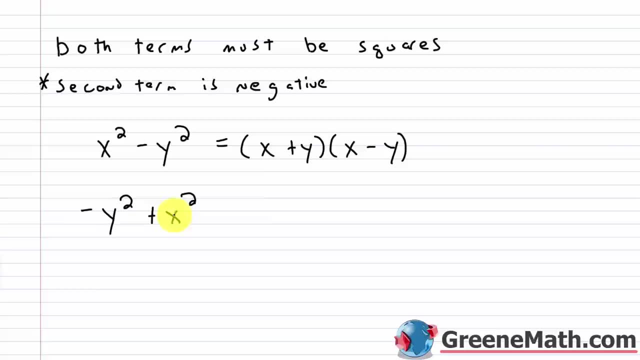 that the second term is negative now. But remember, I could reorder these, I could change this into this and it would still factor the same way. So just pay close attention to that. You want one of the terms to be negative. So those are the two conditions. All right, so let's start out with an. 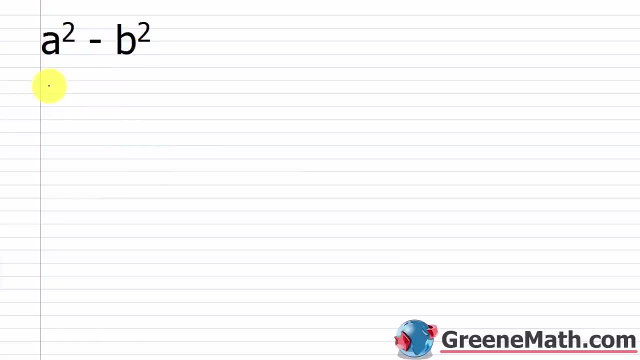 easy one. So we have a squared minus b squared, So we have a squared term here and a squared term here, And then we have a positive and we have a negative. So that's exactly what we're looking for Now. we just follow the format We take. remember when we had x squared minus y squared? 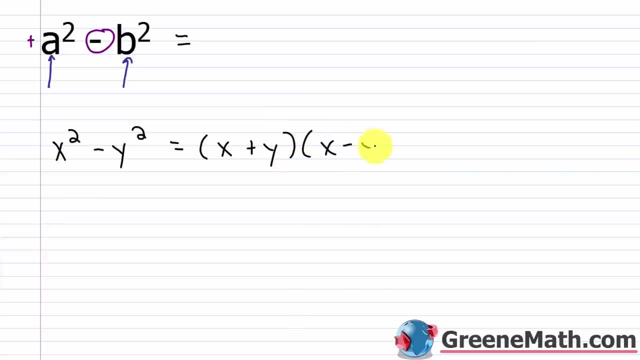 this was x plus y times, x minus y, So you can kind of think about it as: OK, what's being squared is going to go in the first position of each. So what's being squared here is the a. So that's going to go in the first position of each. And then notice your. 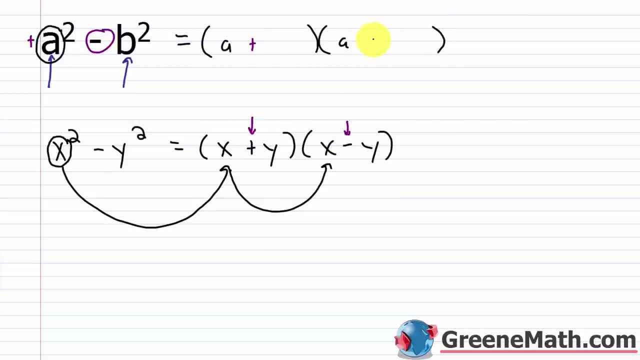 signs. You have different signs, plus and minus, So you'll have plus and minus. And then look at what's squared. here You have y, So that's going to go in your second position of each Same thing. here This b, here is squared, So that's going to go here and here. So a squared, minus b squared. 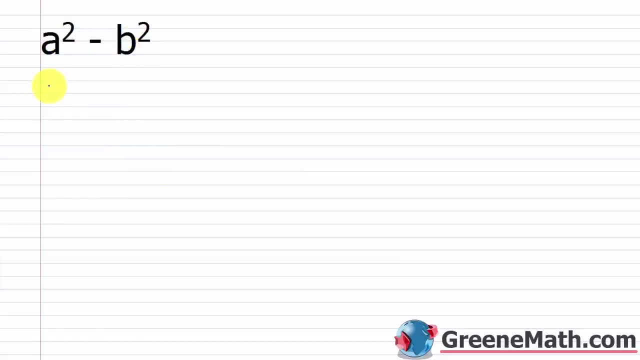 easy one. So we have a squared minus b squared. So we have a square term here, and a square term here. And then we have a positive, and we have a negative. So that's exactly what we're looking 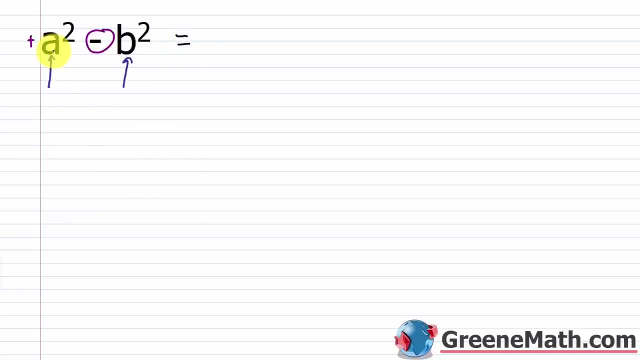 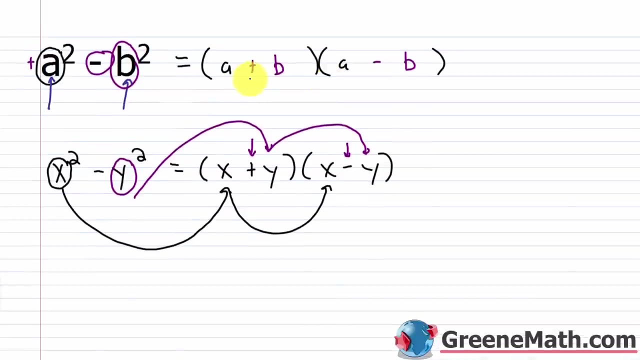 for. Now we just follow the format. We take remember, when we had x squared, minus y squared, this was x plus y squared. So we have a square term here, and a square term here. And then we have a negative y squared plus y times x minus y. So you can kind of think about it as, okay, what's being squared is going to go in the first position of each. So what's being squared here is the a. So that's going to go in the first position of each. And then notice your signs, you have different signs, plus and minus. So you'll have plus and minus. And then look at what's squared here, you have y. So that's going to go in your second position of each. Same thing here, this b here is squared. So that's going to go here, and here. So a squared minus b squared is going to factor into a plus b, that quantity, times a minus b. And so we've already seen this so many times with our special products formulas, we already know that this goes back to this, right? So we don't even need to check it. 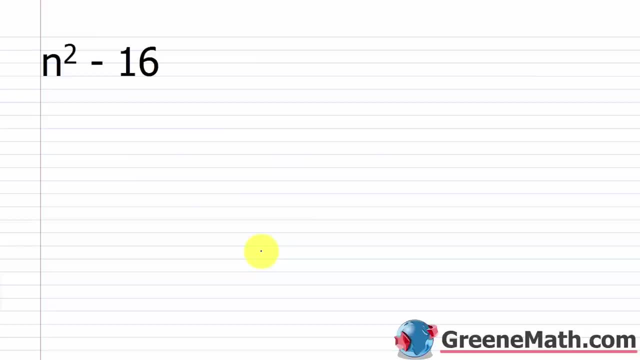 So let's take a look at one that's a little bit harder. So we have n squared minus 16. So we're looking for two squares here. So we know this is a square. And then what about 16? Well, yeah, this is four times four. So I'm going to rewrite this for my convenience as n squared minus four squared. That makes it easier for me to follow that formula. Again, I'm going to write this a few times, x squared minus y squared is equal to x plus y times x minus y. So then this is just equal to what it's equal to n plus four times n minus four, right following that format. Whatever squared here in the first position goes in the first position here and here. Then whatever squared here in the second position goes in the second position here and here. And just remember to alternate your signs. It's just that easy. And again, we know from our special products formula that n plus four, that quantity, times n minus four, that quantity, would give us n squared minus 16. All right, what about x squared minus 25? We know this is a square. And then 25, we know that's five times five. 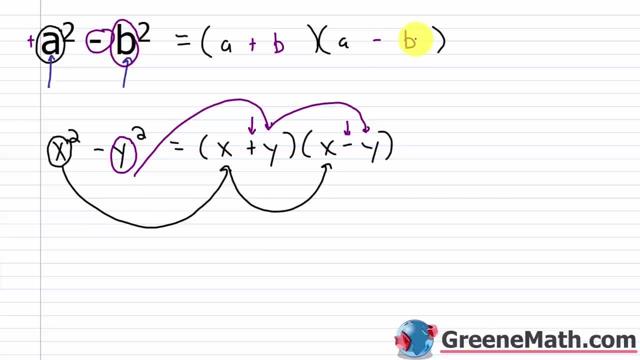 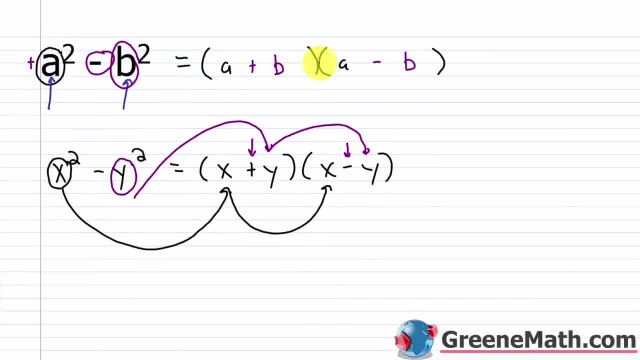 is going to factor into a plus b, that quantity times a minus b, And so we've already seen this so many times with our special products formulas. We already know that this goes back to this- All right, so we don't even need to check it. So let's take a look at one. that's a little bit. 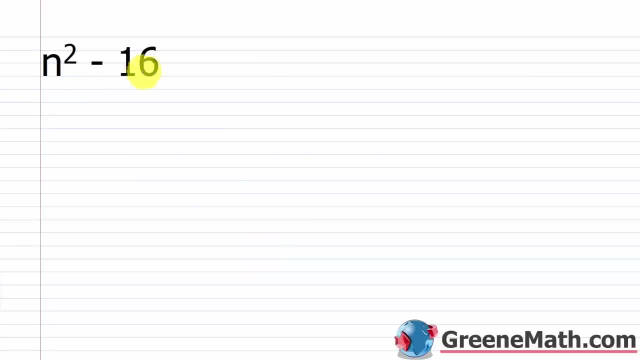 harder. So we have n squared minus 16.. So we're looking for two squares here. So we know this is a square, And then what about 16?? Well, yeah, this is 4 times 4.. So I'm going to rewrite this. 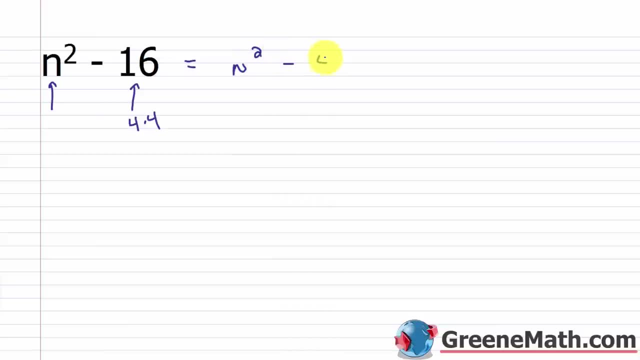 for my convenience, as n squared minus 16.. So I'm going to rewrite this, for my convenience, as n squared squared minus 4 squared. That makes it easier for me to follow that formula Again. I'm going to write this a few times: x squared minus y squared is equal to x plus y times x minus y. So then this: 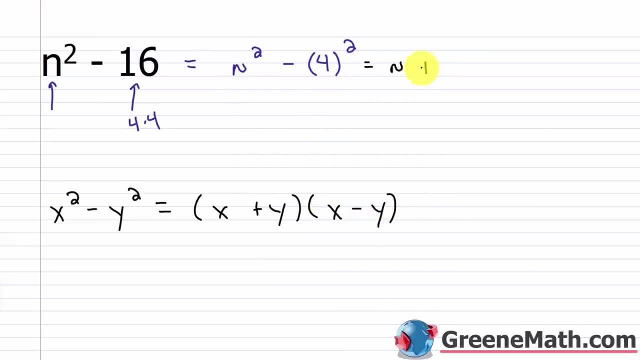 is just equal to what. It's equal to n plus 4 times n minus 4, right, Following that format. Again, whatever squared here in the first position goes in the first position, here and here. Then whatever squared here in the second position goes in the second position, here and here, And just. 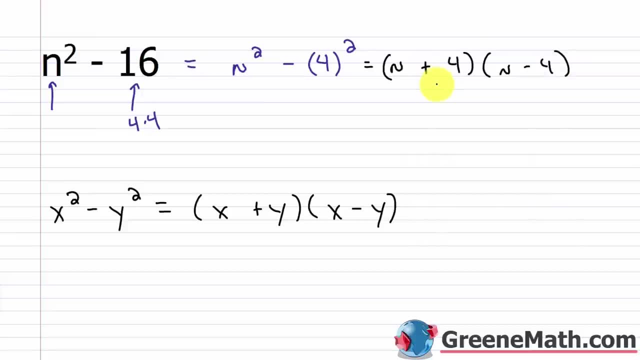 remember to alternate your signs. It's just that easy. And again, we know from our special products formula that n plus 4, that quantity times n minus 4, that quantity would give us n squared minus 16.. All right, what about x squared minus 25?? We know this is a square, and then 25, we know. 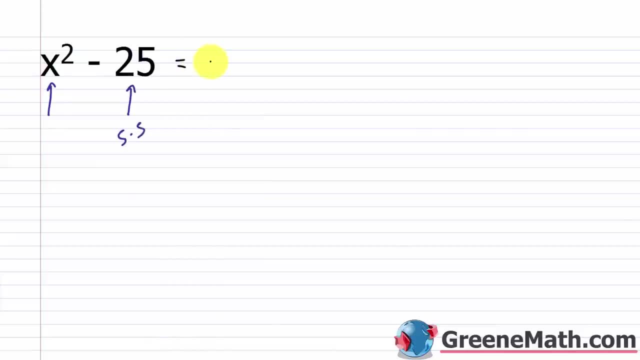 that's 5 times 5.. So again you can rewrite this: x squared minus 5 squared. Again, just follow your formula. If you want, I'll just rewrite it every time. So x squared minus y squared is equal to what x plus y times x. 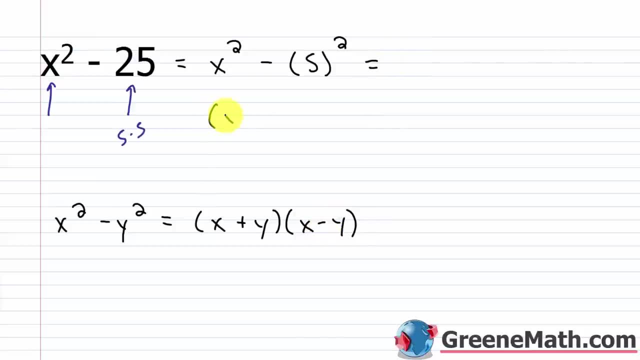 minus y. So then this is equal to what It's x plus 5 times x minus 5, right? Whatever squared in the first position goes here and here, in the first positions of each. Whatever squared in the first position goes here and here, in the first positions of each. 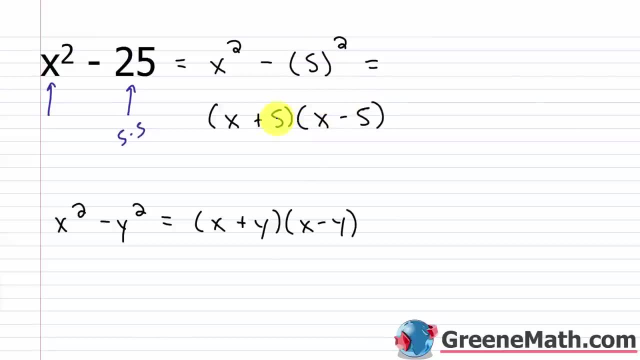 squared in the second position goes here and here in the second position of each, and then again, you know how to check this. you have your special products formulas. we know that the quantity x plus 5 times the quantity x minus 5 would give us x squared minus 25. all right, let's take it up a. 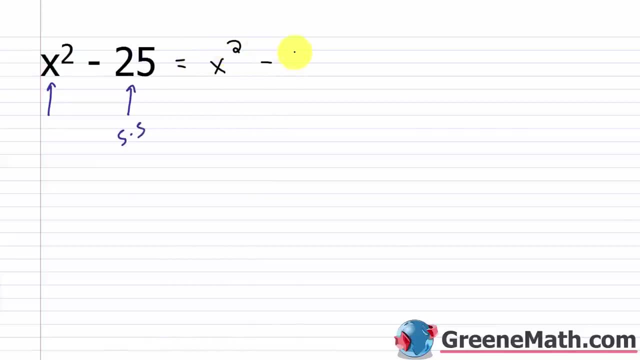 So again, you can rewrite this x squared minus five squared. Again, just follow your formula. If you want, I'll just rewrite it every time. So x squared minus y squared is equal to what? x plus y times x minus y. So then this is equal to what? It's x plus five times x minus five, right? Whatever squared in the first position goes here and here in the first positions of each. 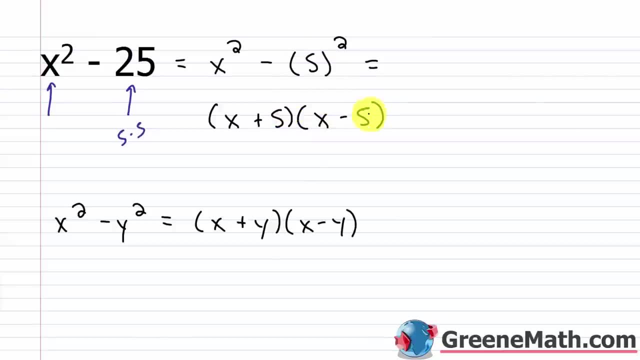 Whatever squared in the second position goes here and here in the first positions of each. And then again, you know how to check this. You have your special products formulas. We know that 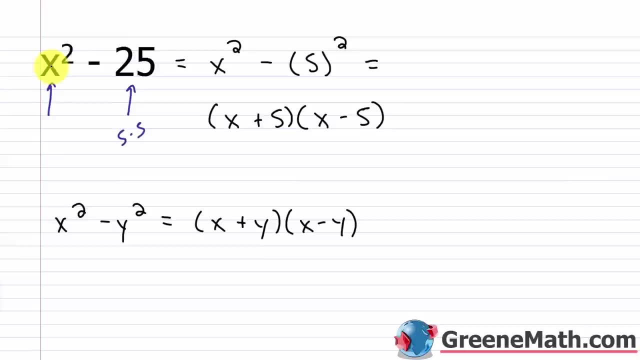 the quantity x plus five times the quantity x minus five would give us x squared minus 25. 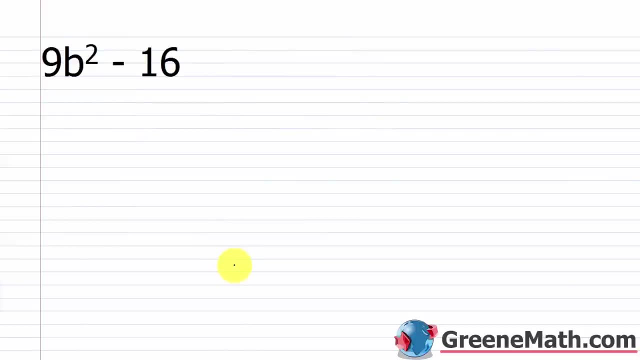 All right, let's take it up a notch. We'll look at one that's a little bit more complicated. So we have nine b squared minus 16. So then this one right here, we know nine is three times three. 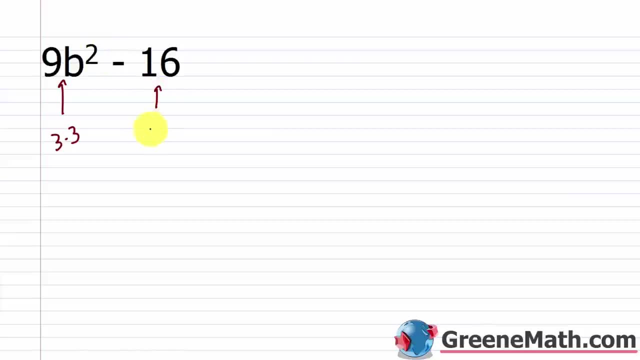 Obviously, b squared is a square. And then 16, we know that's four times four. 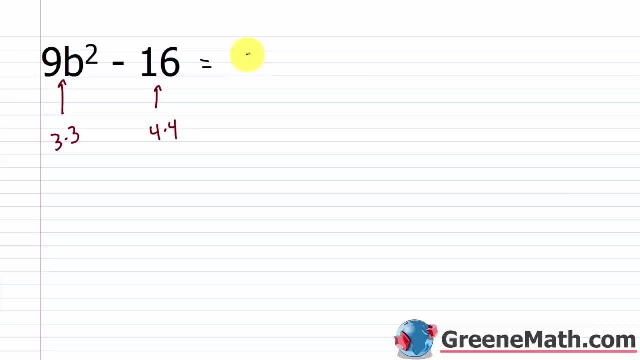 So again, to follow that kind of formula, I can write this as three b, that quantity squared minus four squared. And then I can write this, remember, whatever's in the first position that's squared is going to go on the first position of each. And then whatever's in the second position that's squared, that's going to go on the second position of each. So this becomes the quantity three b plus four. Times the quantity three b minus four. And again, if you want to check this, you know your formula already. It'd just be first times first. Three b times three b is nine b squared. And then you know that the middle terms would drop out. So the outer and the inner would go away. You just need to think about the last. You have plus four times negative four. That's going to be negative 16. 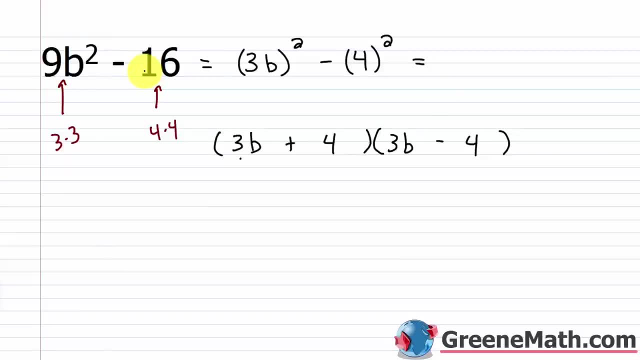 So you would get nine b squared minus 16 back. All right, let's take a look at another one. So we have 125 x minus 80 x cubed. 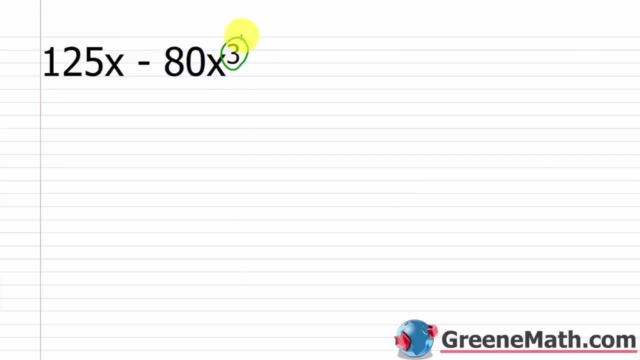 So we'll see this cubed here and say, well, this isn't the difference of two squares. 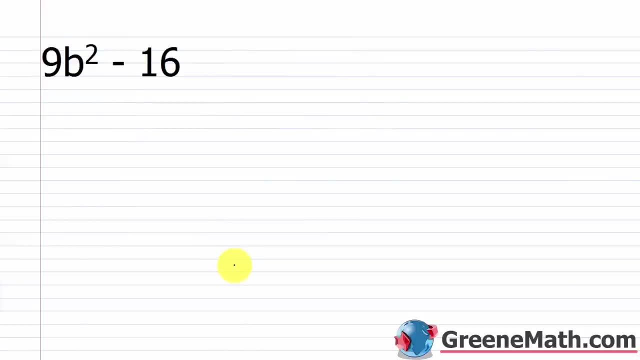 notch. we'll look at one that's a little bit more complicated. so we have 9b squared minus 16. so then this one: right here, we know 9 is 3 times 3. obviously b squared is a square. and then 16, we know that's 4 times 4. so again, to follow that kind of formula, I can write this as 3b, that quantity. 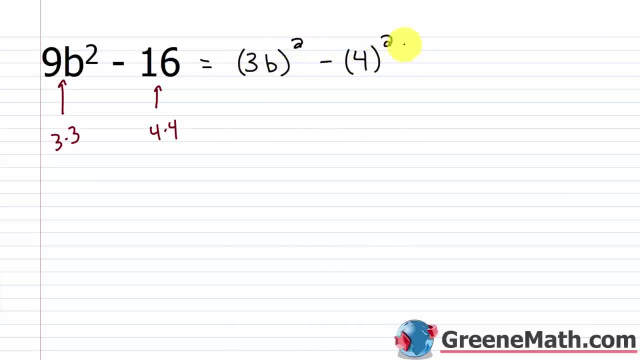 squared minus 4 squared. and then I can write this: remember, whatever's in the first position that's squared is going to go on the first position of each, and then whatever's in the second position that's squared, that's going to go in the second position of each. so this becomes: 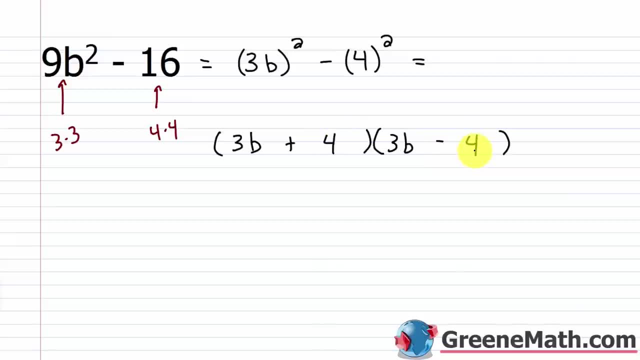 the quantity x squared minus 4 times 4. so again, to follow that kind of formula, I can write this as 3b plus 4 times the quantity 3b minus 4. and again, if you want to check this, you know your formula already. it'd just be first times first. 3b times 3b is 9b squared, and then you know that the middle. 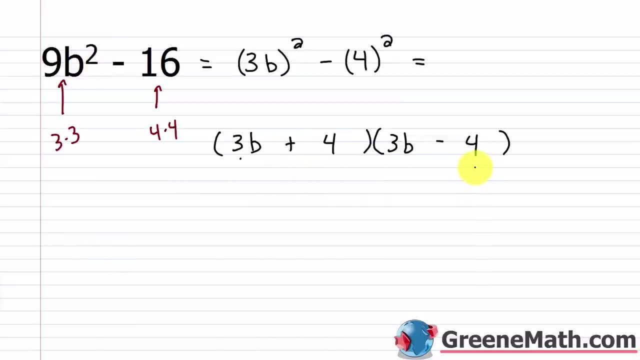 terms would drop out. so the outer and the inner would go away. you just need to think about the last you have, plus 4 times negative 4, that's going to be negative 16. so you would get 9b squared minus 16 back. all right, let's take a look at another. so we have 125x minus 80x cubed. 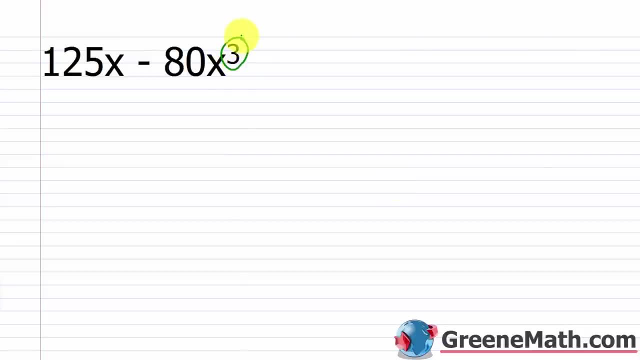 now a lot of you will see this cubed here and say: well, this isn't the difference of two squares. i want you to remember something whenever you factor. you want to think about what's common to everything before you even start. so i would think about: okay, both terms here have an x. 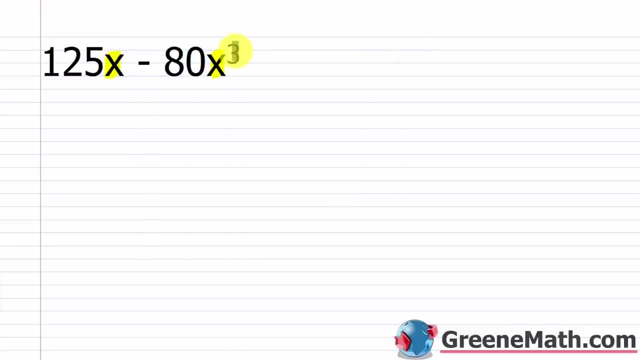 right, at least one. this one's obviously got three x times x times x, but this one has one and this one has at least one. Then both of these guys are divisible by five. This is 16 times five and this is 25 times five. Now, when you see that, you can see that 25 is five times five and 16 is. 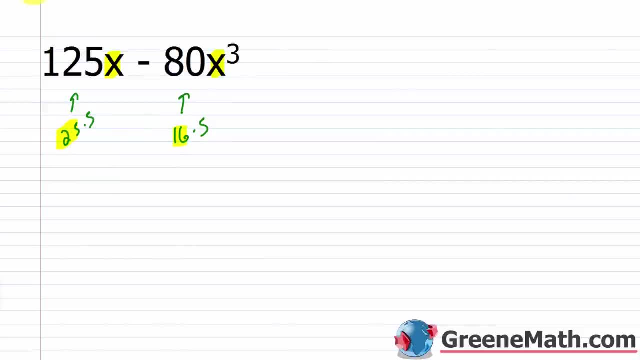 four times four. So this looks like the perfect kind of trap question. you get on a test. What they want you to do is they want you to factor out the GCF first. So the GCF is 5x. So if I pulled, 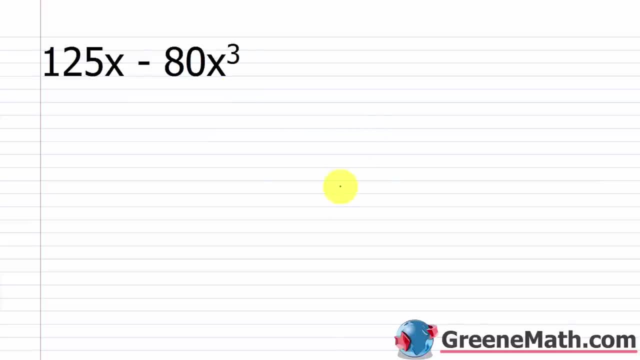 I want you to remember something. Whenever you factor, you want to think about what's common to everything before you even start. So I would think about, okay, both terms here have an x, right? At least one. This one's obviously got three, x times x times x. But this one has one, and this one has at least one. Then both of these guys are divisible by five. This is 16 times five. And this is 25 times five. Now, when you see that, you can see that 25 is five times five, and 16 is four times four. So this looks like the perfect kind of trap question you get on a test. 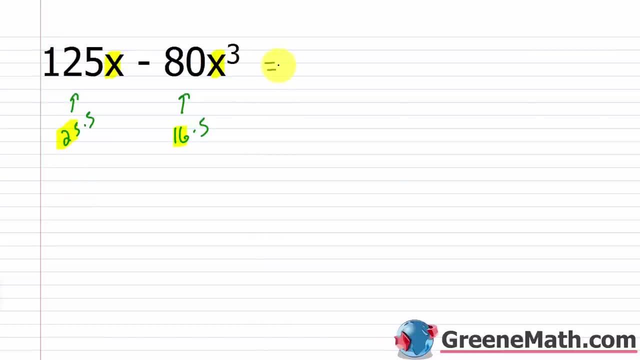 What they want you to do is they want you to factor out the GCF first. So the GCF is five x. So if I pulled that out, what I'd have left, 125 x divided by five x is going to be 25, and then minus, then 80 x cubed. So 80 cubed divided by five x would give me 16 x squared. Now, this isn't in the format that we're used to. We're used to a variable here or something like that, but we still have something that's squared minus something else that's squared, right? So that's exactly what we're looking for. Let me erase all this. And again, we're putting our five x out in front, and then we'll set up two parentheses here. And so 25 is what? It's five times five. So we would have five and five here. And then we have a plus and a minus. 16 x squared, we can think of as four x times four x. 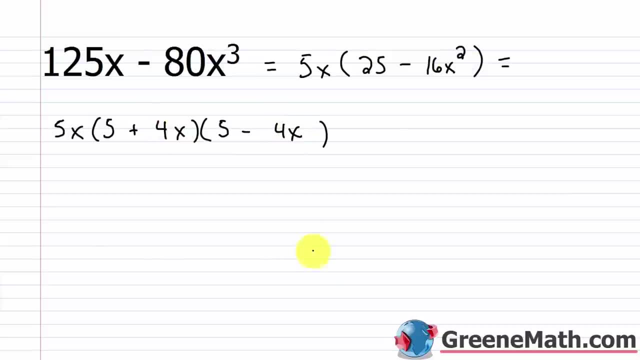 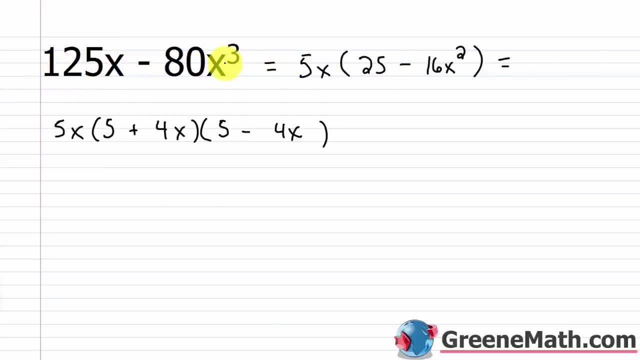 and then we would get back to 125 x minus 80 x cubed. So now let's take a look at something else that's very common. We're going to look at some perfect square trinomials. So perfect 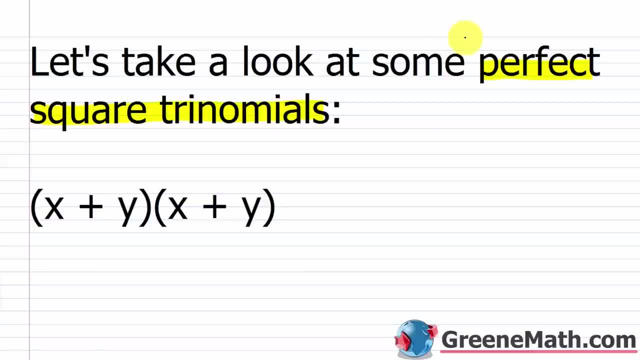 square trinomials. So in other words, a trinomial, again, is a polynomial with three terms, and it factors into a binomial that's squared. So in other words, this guy right here, we already know the formula for this. This is x squared plus two x y plus y squared. 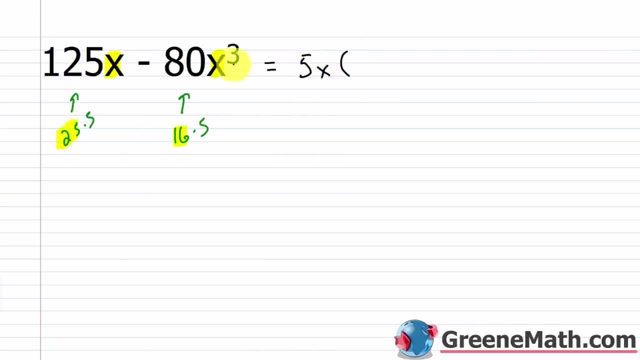 that out, what I'd have left- 125x divided by 5x- is going to be 25, and then minus, then 80x cubed divided by 5x would give me 16x squared. Now, this isn't in the format that we're used to. We're used. 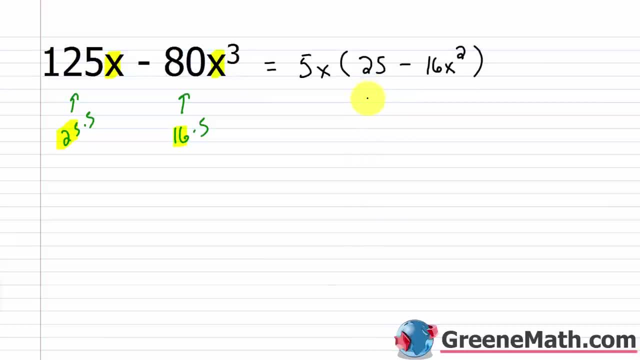 to a variable here or something like that, but we still have something that's squared minus something else that's squared. So that's exactly what we're looking for. Let me erase all this, and again we're putting our 5x out in front, and then we'll set up two parentheses here, and so 25 is what It's: five. 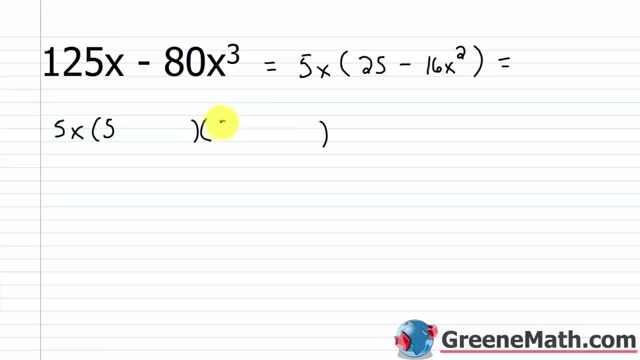 times five. So we would have five here and five here and then we have a plus and a minus. 16x squared we can think of as 4x times 4x. So I'll put 4x here and 4x here and if you go through and 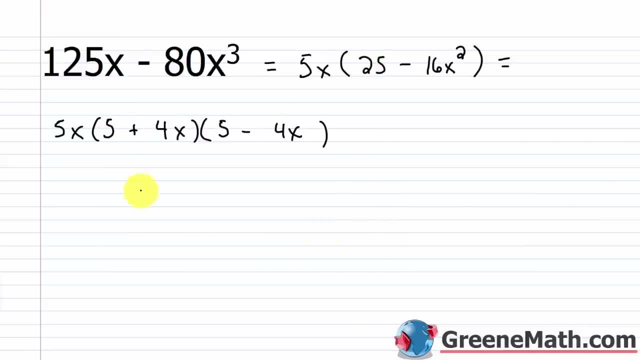 you do FOIL five times five is 25.. The outer which is negative, 20x, and the inner, positive 20x, would cancel, and then the final 4x times negative. 4x is negative 16x squared. So that checks out. and if we multiplied this by 5x we would get back to 125x minus 80x cubed. So now 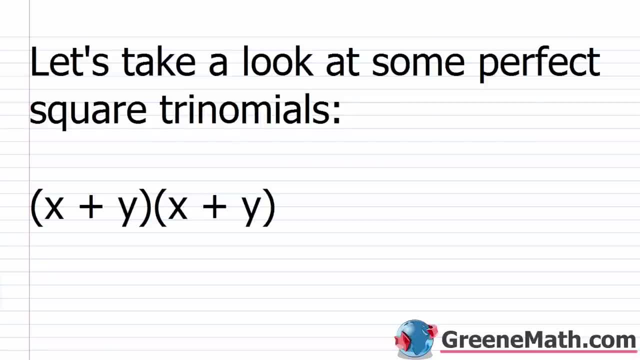 let's take a look at something else that's very common. We're going to look at some perfect square trinomials. So perfect square trinomials. So in other words, a trinomial again is a polynomial with three terms and it factors into a binomial. 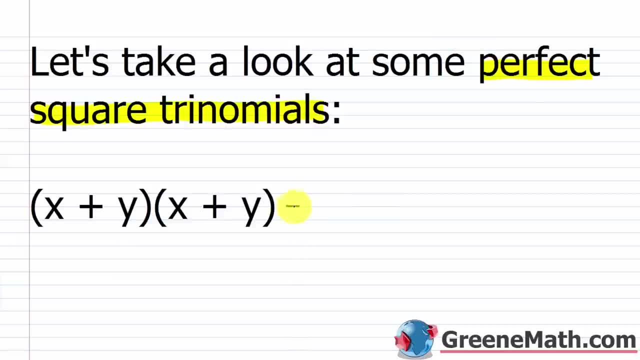 That's squared. So in other words, this guy right here. we already know the formula for this. This is x squared plus 2xy plus y squared. So if I factored it into this, really I could write this as the quantity x plus y squared. Right, these two would be the same. So if we see something like: 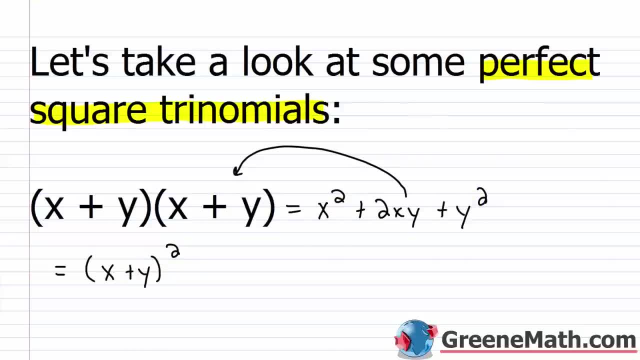 this in this format and we notice that we have the first guy squared and the last guy squared and then the middle guy squared. So we have the first guy squared and the middle guy squared. The middle is two times both of the terms in the squared binomial, So 2 times x times y. Well, we have. 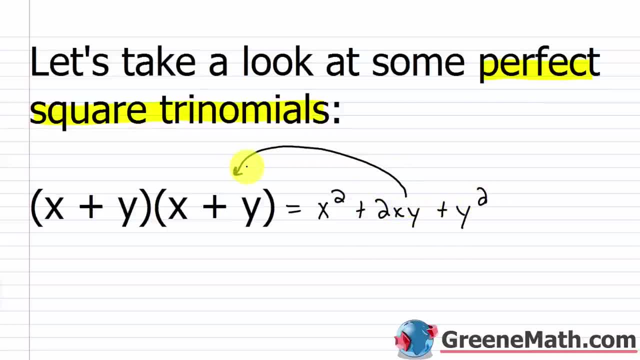 So if I factored it into this, really, I could write this as the quantity x plus y squared, right? These two would be the same. So if we see something like this in this format, and we notice that we have the first guy squared and the last guy squared, and then the middle is two times both of the terms in the squared binomial, so two times x times y, well, we have a perfect square trinomial. 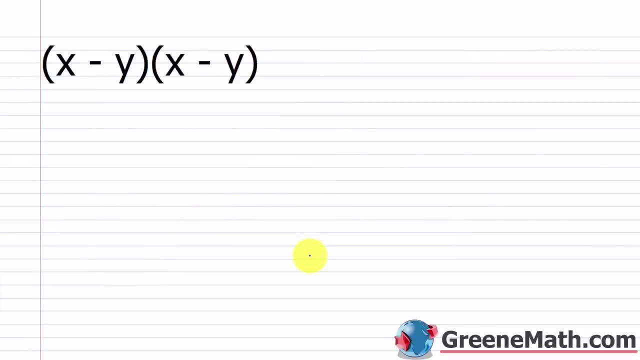 And we can factor it using this formula. So another occurrence of this, we have x minus y times x minus y. And so again, this is x minus y, that quantity squared. We already know this turns into x squared. We have a minus sign here, then two x y, and we have a plus, and then y squared. So same thing, just when you have a negative there, that sign right there is going to be negative. If I have the x plus y, that quantity squared, all the signs are positive. 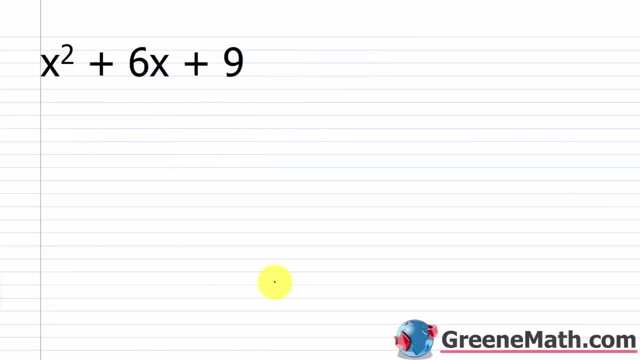 But everything else, all the terms are the same. All right, so let's take a look at the first example. So we have x squared plus 6x plus 9. So again, the first thing I'm going to look at is to see if this is a square. So yeah, this is x squared. And then is this a square? Well, this is 3 squared. Now, the next thing I'm going to look at is the middle term. If I multiplied 3, which is what's squared here, times x, which is what's squared here, so 3 times x is 3x, times 2, do I product? I do. 2 times 3 is 6. 6 times x is 6x. So then I can factor this guy as this, what's squared, which is x, plus this, which squared, which is 3, that whole quantity squared. All 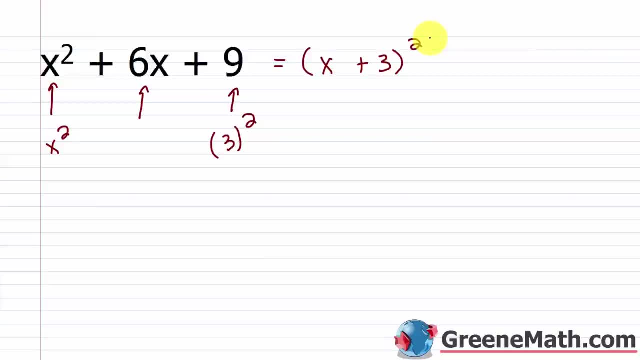 right, this turns into x plus 3, that quantity, times x plus 3. All right, let's take a look at 25p squared minus 30p plus 9. Now, pay attention here, because we have that minus sign. So we know if this ends up being factorable, there's going to be a minus sign in there. You'll have something minus something else, and then it'll be squared. So let's check to see if we have squares here. So 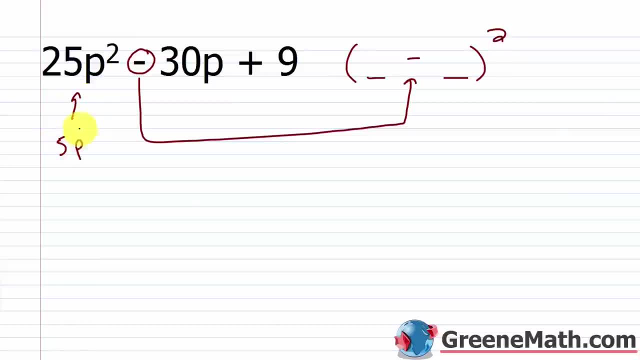 we have 25p squared. So that's 5p, that amount squared. And then we have 9. That's 3 squared. 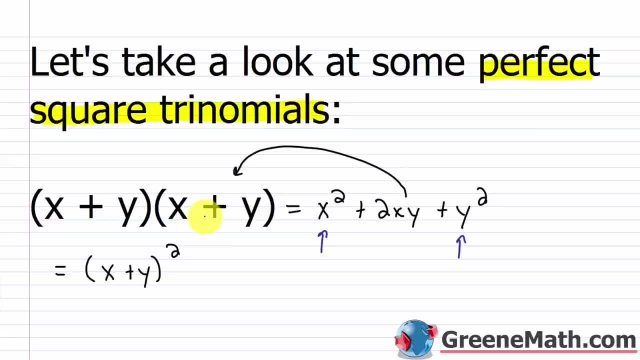 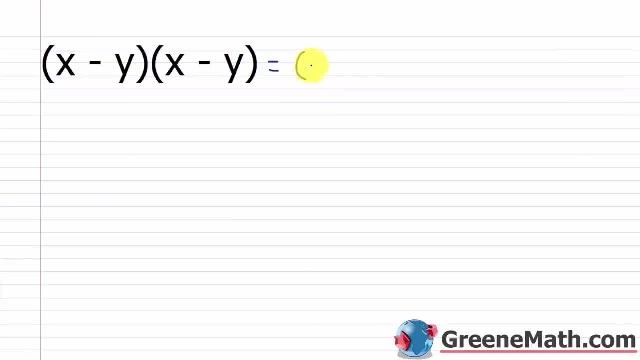 a perfect square trinomial and we can factor it using this formula. So another occurrence of this: we have x minus y, times x minus y, And so again this is x minus y, that quantity squared. We already know this turns into x squared. We have a minus sign here, then 2xy, and we have a plus and then y. 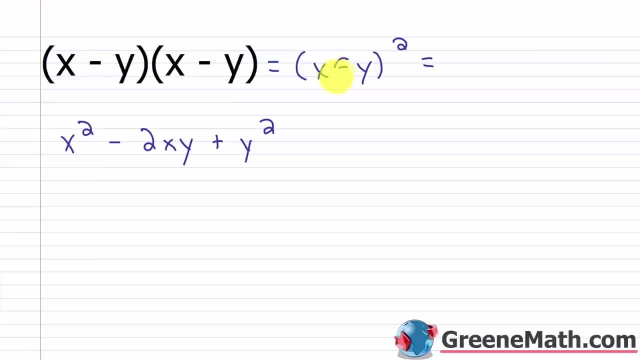 squared Same thing. just when you have a negative there, that sign, right there, is going to be negative. If I have the x plus y, that quantity squared, all the signs are positive, But everything else, all the terms are the same. All right, so let's take a look at the first example. So we have x squared plus 6x. 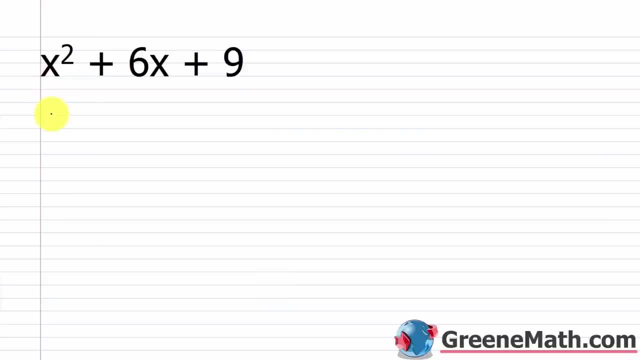 plus 9.. So, again, the first thing I'm going to look at is to see if this is a square. So yeah, this is x squared. and then is this a square? Well, this is 3 squared. Now, the next thing I'm going to look at 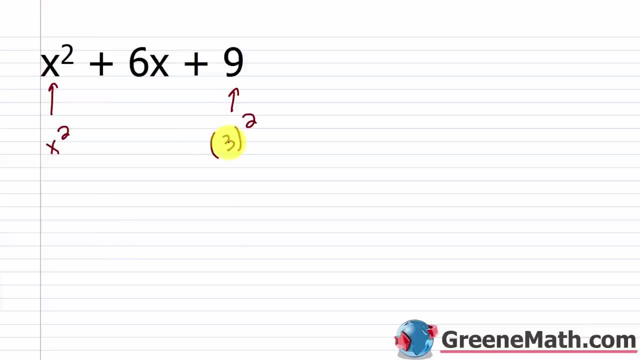 is the middle term. If I multiplied 3, which is what's squared here, times x, which is what's squared here, So 3 times x is 3x times 2, do I get the middle product I do: 2 times 3 is 6.. 6 times x is 6x, So then I can factor this guy as this. 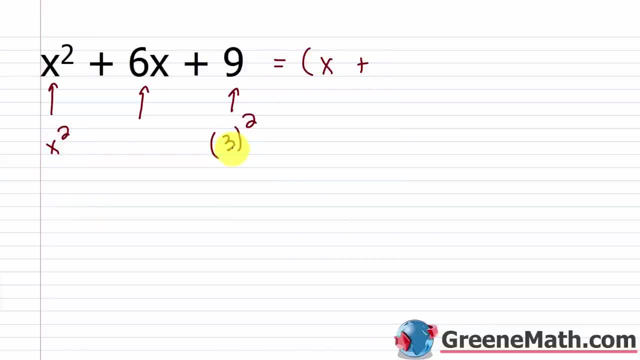 what's squared which is x plus this, which squared which is 3.. That whole quantity squared. All right, this turns into x plus 3, that quantity times x plus 3.. All right, let's take a look at 25p squared minus 30p plus 9.. Now pay attention here, because we have 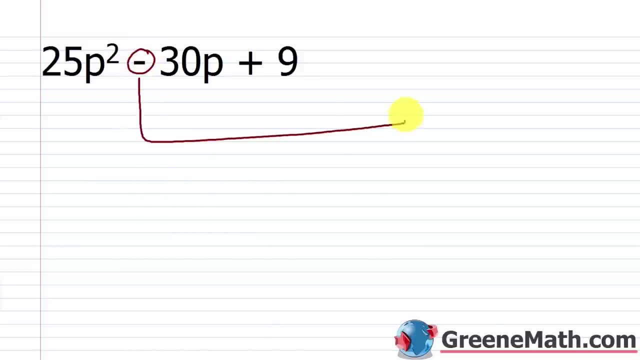 that minus sign. So we know that if this ends up being factorable, there's going to be a minus sign in there. You'll have something minus, something else and then it'll be squared. So let's check to see if we have squares here. So we have 25p squared, So that's 5p, that amount squared, and 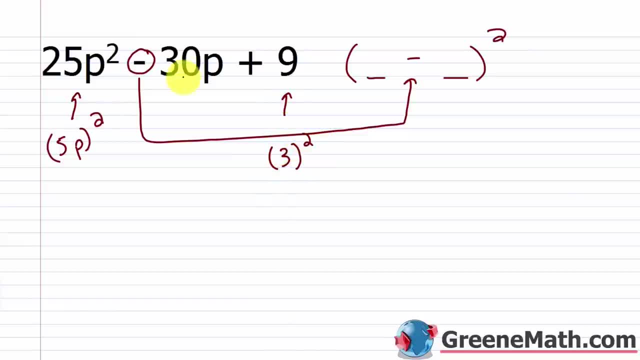 then we have 9.. That's 3 squared. And then what about 5p squared? That's 5p squared, That's 3 squared. So what about our middle product? Is it 2 times 5p times 3?? 2 times 3 is 6.. 6 times 5 is 30.. 30 times. 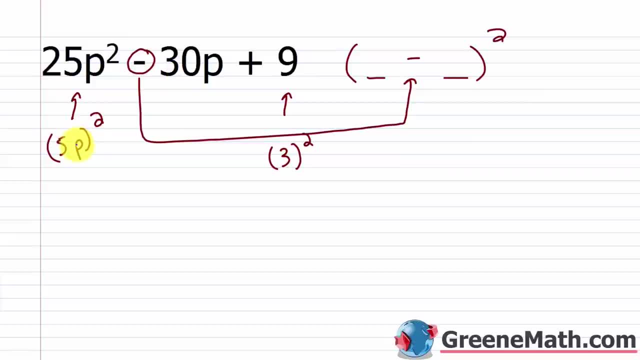 p is 30p. So yes, that all works out. So we would write this: We take what's being squared in the first term, So that's 5p. That goes in the first position, And then, minus we take what's squared. 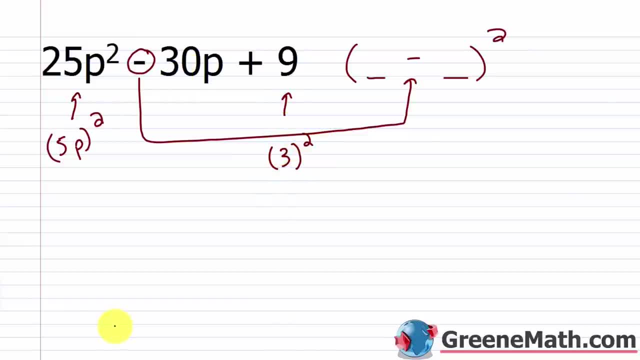 And then what about our middle product? Is it 2 times 5p times 3? 2 times 3 is 6. 6 times 5 is 30. So yes, that all works out. So we would write this. We take what's being squared in the first term. So that's 5p. That goes in the first position. And then minus, we take what's squared 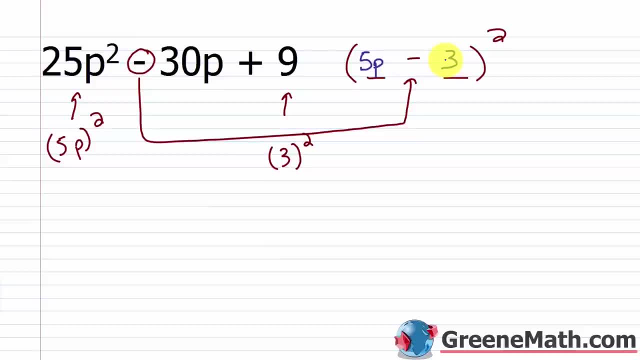 in the last position, that 3, and we write that. So you get the quantity 5p minus 3. That's squared. 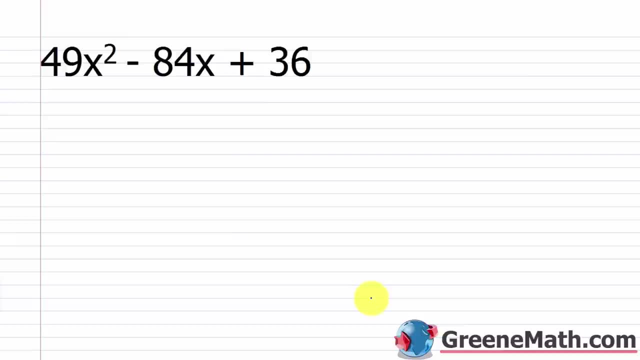 All right, let's take a look at another one. So we have 49x squared minus 84x plus 36. So this guy right here, you think about 49, that's 7 times 7. And then x squared is x squared. So that's 7x, that guy squared. And then for 36, we think about that as 6 squared, right? 6 times 6. 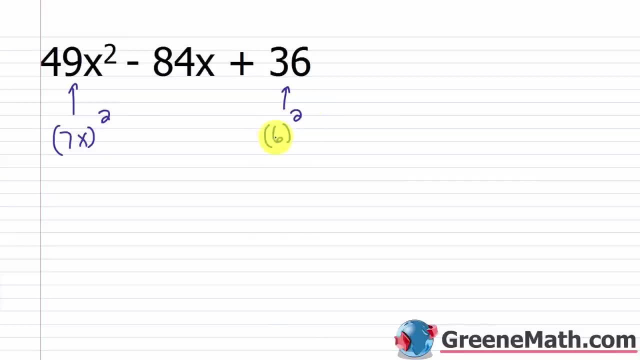 So is the middle term 2 times the product of 6 times 7x? 2 times 6 is 12. 12 times 7 is in fact 84. And the x would come along for the ride. So that would give you 84x. Now there's a minus sign here. So when you set this up, it's going to be this guy here, 7x. 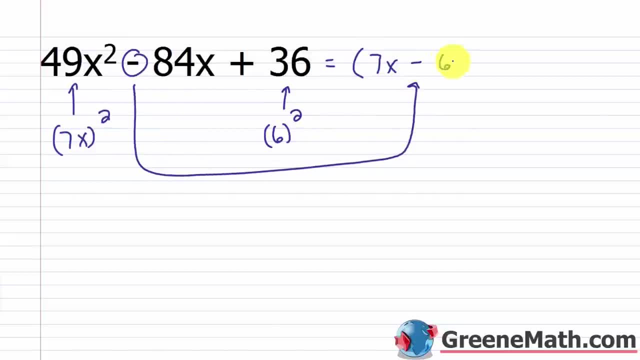 There's a minus. And then this guy right here, 6. So this amount, this quantity, squared. All right, let's take a look at another one. So we have 72x cubed plus 120x squared plus 50x. So the first 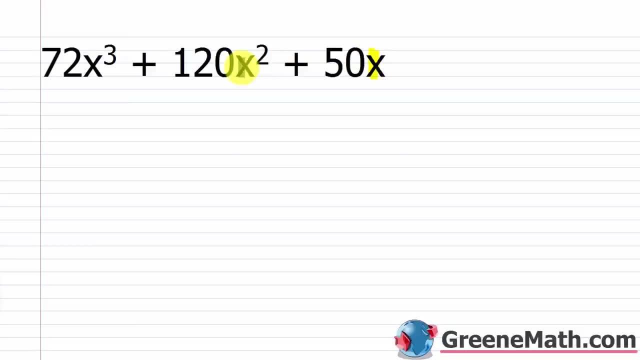 thing I noticed right away is that everything has an x, right? That's common to everything. 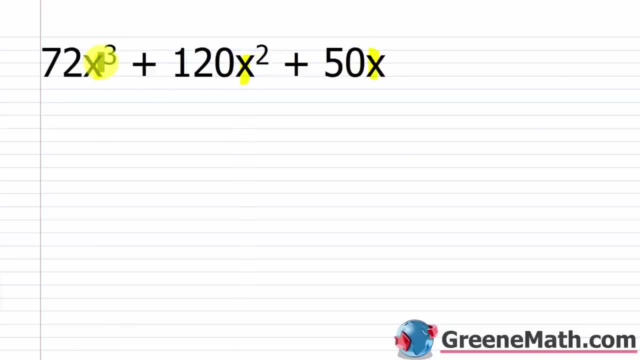 Now everything is also divisible by 2. So I can pull out a 2x before I even begin. And what that's going to give me is 36x squared. 6x squared plus 60x plus 25. And I notice right away that 36 is what? It's 6 times 6. So this would be 6x, that amount squared. 25 I know is 5 squared. And then for your middle term, 2 times 5 is 10. 10 times 6 is 60. x comes along for the ride. So I would get 60x. Now all I need to do, again, make sure you have that 2x out in front. 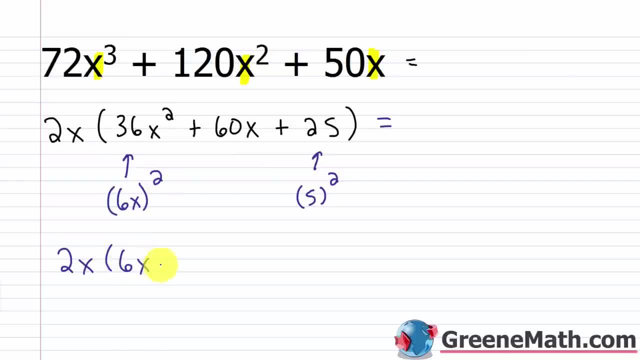 I would put 6x in the front. I would put 6x in the first position. I have 2 plus signs here. So this is going to be plus. 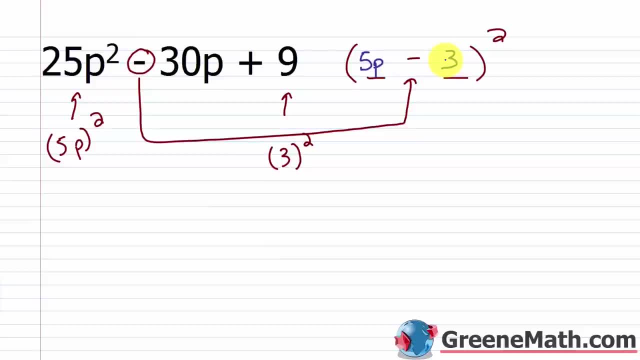 in the last position that 3 and we write that. So you get the quantity 5p minus 3.. That's squared. All right, let's take a look at another one. So we have 49x squared minus 84x plus 36.. So this guy right here you think about 49. that's 7 times 7.. 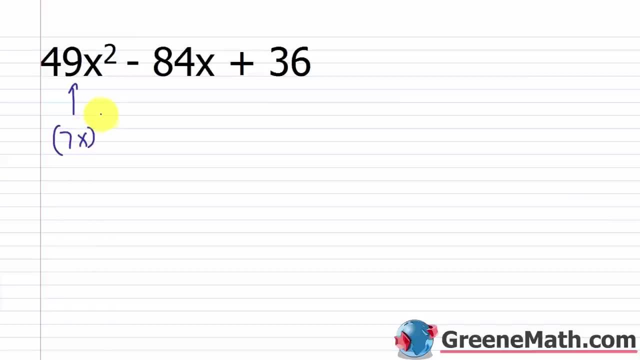 And then x squared is x squared, So we'll put 7x, that guy squared, And then for 36 we think about that as 6 squared, Right, 6 times 6.. So is the middle term 2 times the product of 6 times 7x. 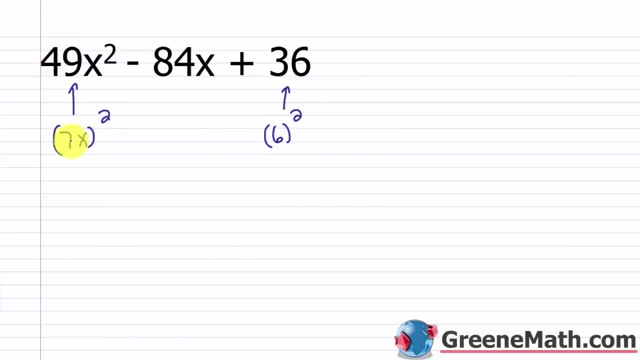 2 times 6 is 12.. 12 times 7 is in fact 84. And the x would come along for the opposite, So that would give you 84x. Now there's a minus sign here, So when you set this up, it's. 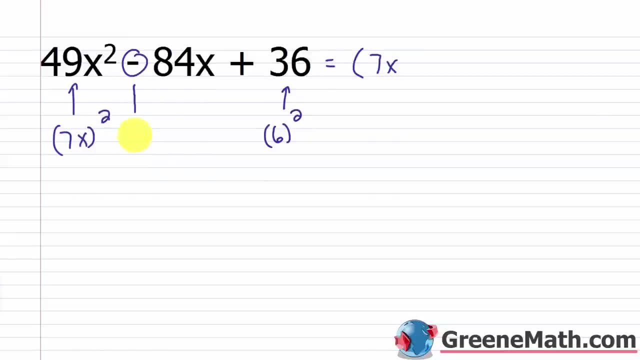 going to be this guy here: 7x, There's a minus, And then this guy right here, 6.. So this amount is quantity squared. All right, let's take a look at another one. So we have 72x cubed plus 120x. 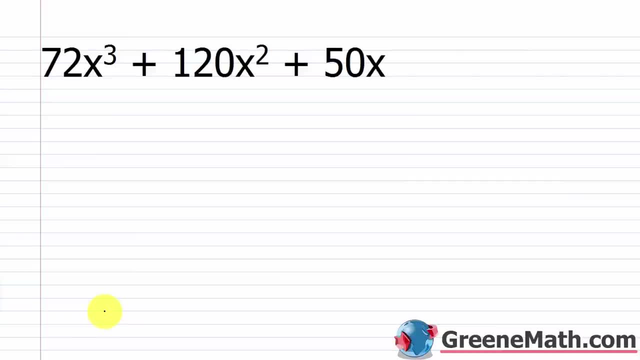 squared plus 50x. So the first thing I noticed right away is that everything has an x Right. that's common to everything divisible by 2, so I can pull out a 2x before I even begin and what that's going to give me is 36 x squared plus 60 X plus 25, and I notice right away that. 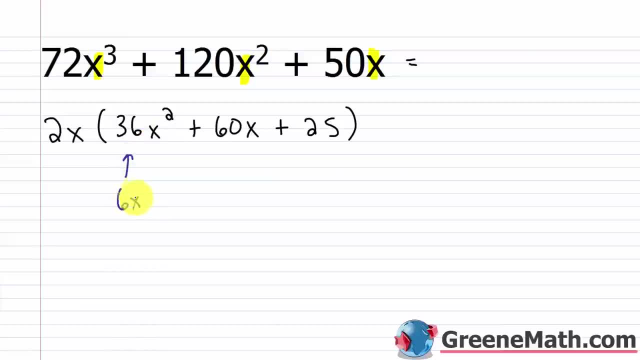 36 is what it's 6 times 6, so this would be 6x. that amount squared, 25, I know, is 5 squared. and then, for your middle term, 2 times 5 is 10, 10 times 6 is 60, X comes. 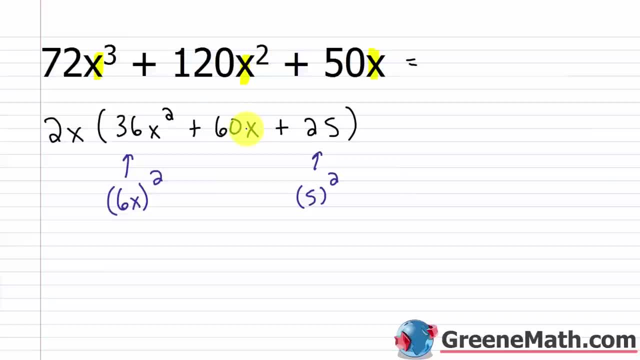 long for the ride, so I would get 60 X. now all I need to do again make sure you have that 2x out in front. I would put 6x in the first position. I have 2 plus signs here, so this is going to be plus, and then I'll put 5 in the second. 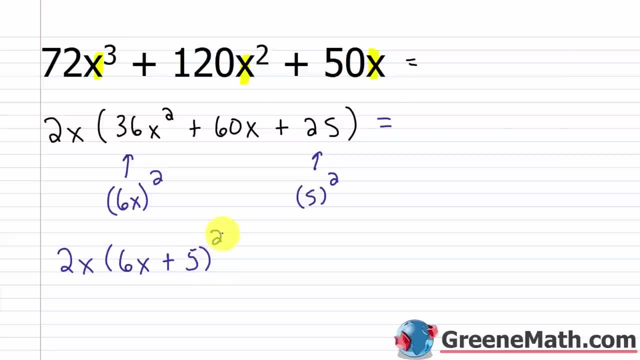 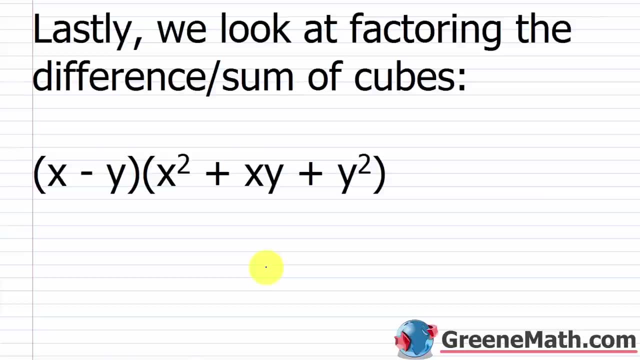 position and then this is squared. so this is going to factor into 2x times a quantity, 6x plus 5, squared, alright. so, lastly, we're going to look at factoring the difference, or also the sum of cubes. now, you, this is one that's going to be confusing for you at first, because when we looked, 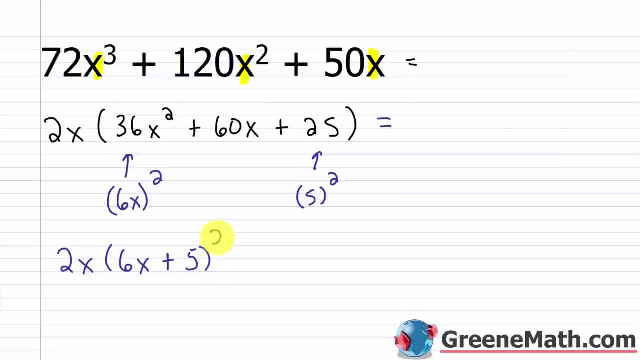 And then I would put 5 in the second position. And then this is squared. So this is going to factor into 2x times a quantity, 6x plus 5 squared. All right, so lastly, we're going to 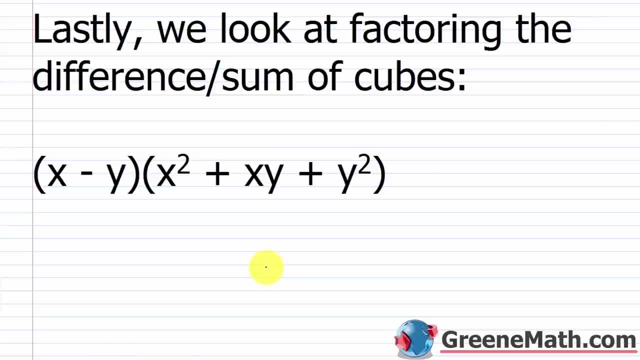 look at factoring the difference or also the sum of cubes. Now this is one that's going to be confusing for you at first because when we looked at our special products lesson, we saw something that was similar, but it's not the same. And I'm going to show you how to do that. So I'm going to 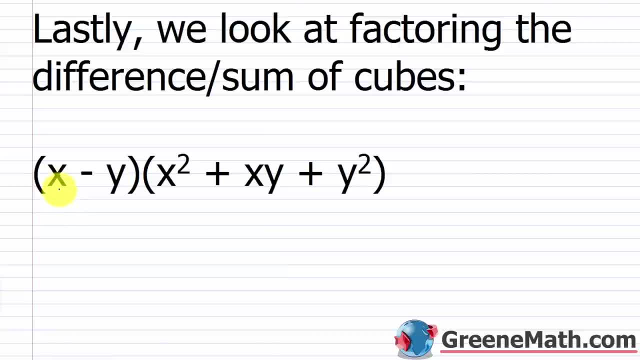 show you that in a minute. Let me go through and just kind of use the distributive property on this and show you what you get. x times x squared is x cubed. x times xy is plus x squared y. 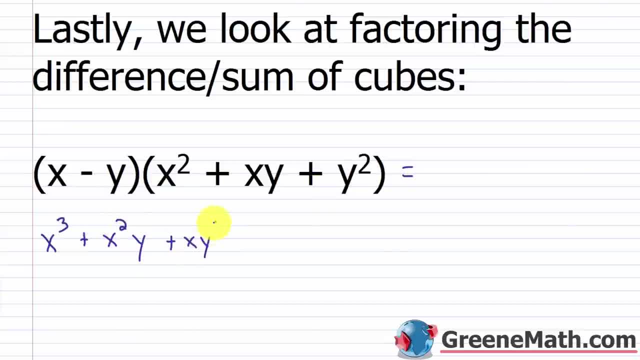 And then x times y squared is plus xy squared. Negative y times x squared is minus x squared y. Negative y times xy is negative xy squared. And then lastly, negative y times y squared is minus y. 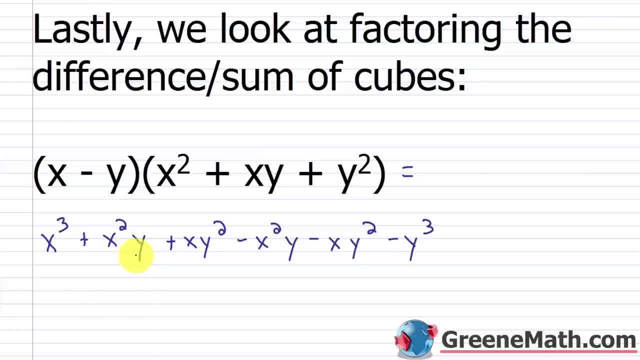 Now what's going to happen is x squared y minus x squared y. Those are going to cancel. Plus xy squared minus xy squared. Those are going to cancel. And what I'm left with is x cubed minus y cubed. So this is one that's going to dramatically speed up your time to do homework 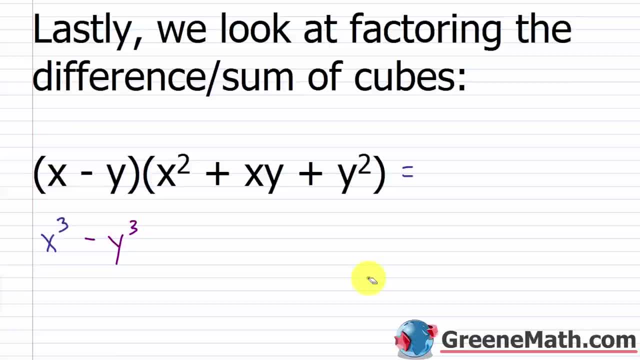 or take a test. So you have to memorize it. It's something you just have to practice, write down on a flashcard, just kind of go through. Now here's what I'm going to tell you. This is not going to be a problem. This is going to be a problem. This is going to be a problem. 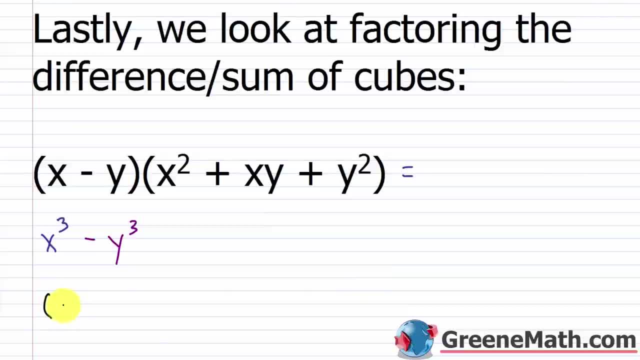 This is not the same as when we looked at the quantity x minus y cubed. Remember, I can't just distribute my exponents and say this is equal to x cubed minus y cubed. No. Wrong. Remember that. 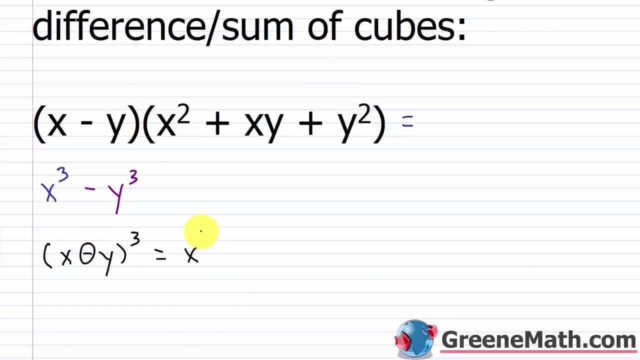 If I have a minus here, I have x cubed. I have a minus here. And then remember, I have a space, a plus, a space, a minus, and then a y cubed. So what goes in these two blanks here? 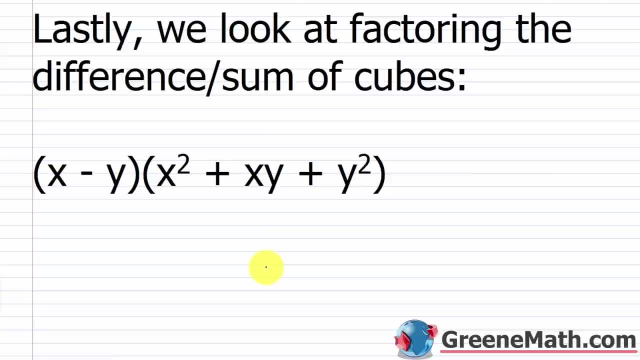 at our special products lesson we saw something that was similar but it's not the same, and I'm going to show you that in a minute. let me go through and just kind of use a distributive property on this and show you what you get. x times x squared is x cubed, x times xy is plus x squared, y and. 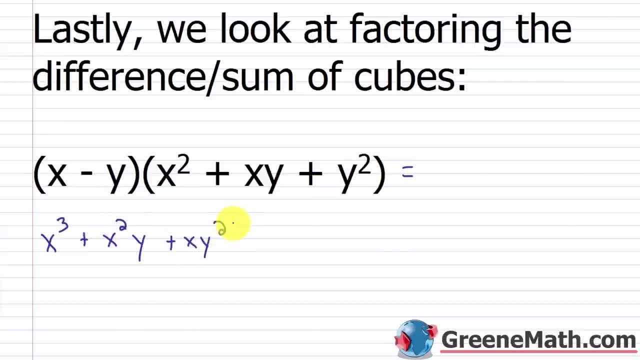 then x times y squared is plus xy squared. negative y times x squared is minus x squared y. negative y times xy is negative xy squared. and then, lastly, negative y times y squared is minus y cubed. now what's going to happen is x squared y minus x squared y. those are going to cancel plus xy squared minus xy. 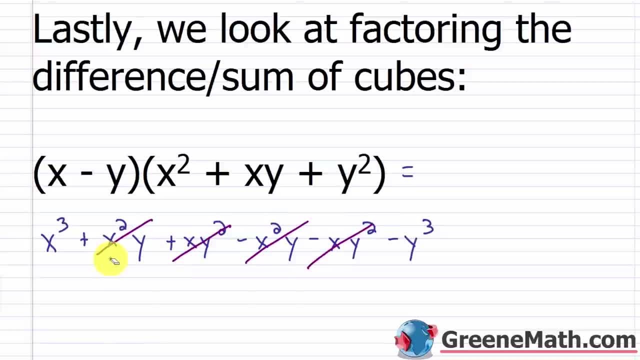 squared, those are going to cancel, and what I'm left with is x cubed minus y cubed. so this is one that's going to dramatically speed up your time to do homework or take a test. so you have to memorize it, it's, it's something you just 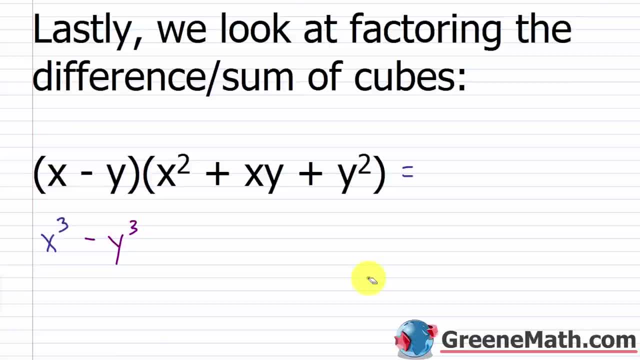 have to practice, write down a flash card, just kind of go through. now here's what I'm going to tell you. this is not the same as when we looked at the quantity x minus y cubed, remember. I can't just distribute my exponents and say this is: 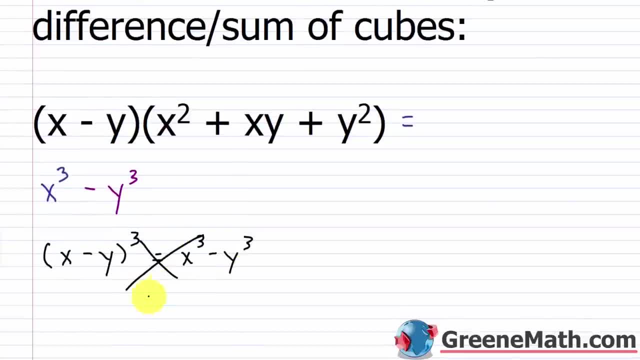 equal to x cubed minus y cubed. no wrong, remember that. okay, these are not the same. I taught you this formula already and it's really easy to remember: if I have a minus here, I have x cubed, I have a minus here, and then remember I have a space a plus a space a. 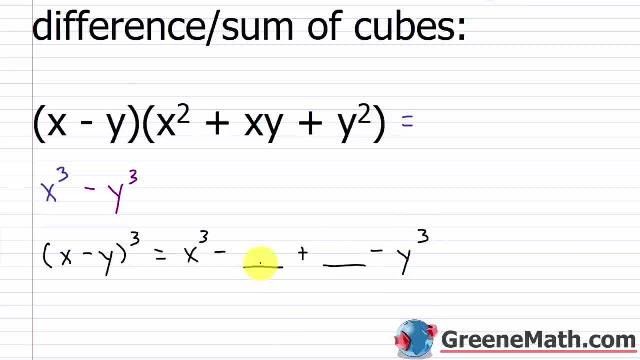 minus and then a y cubed. so what goes in these two blanks here? this is a 3 and this is a 3, remember from the exponent. and then each term goes in there. each one is squared only once. so in other words, I would do x squared y here and 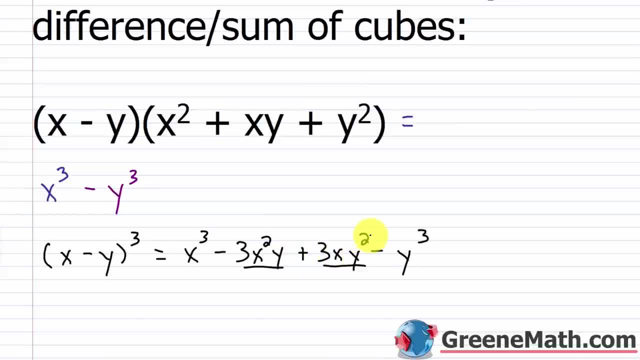 and I'll do xy squared here. So this is what this is equal to and this is what this is equal to. They are not the same. So please understand that, because a lot of students will see something like this and they'll try to factor it into this. 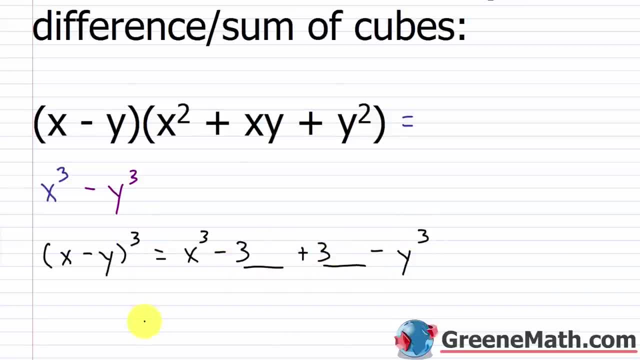 This is a three and this is a three. Remember that from the exponent. And then each term goes in there. Each one is squared only once. So in other words, I'll do x squared y here and I'll do x y squared here. So this is what this is equal to. And this is what this is equal to. 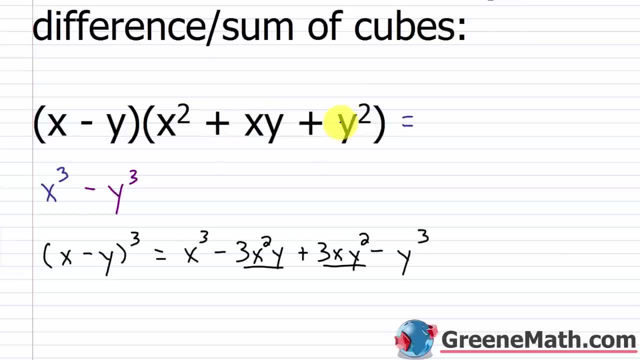 They are not the same. So please, understand that because a lot of students will see something like this and they'll try to factor it into this. It's not the same. Okay. So please understand that. This formula was something we 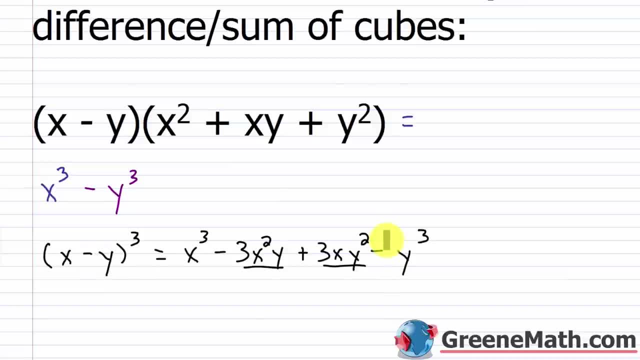 talked about when we looked at special products. So let me erase this real quick. And I want to show you the sum of cubes. So this is the difference of cubes. This, again, is the difference. 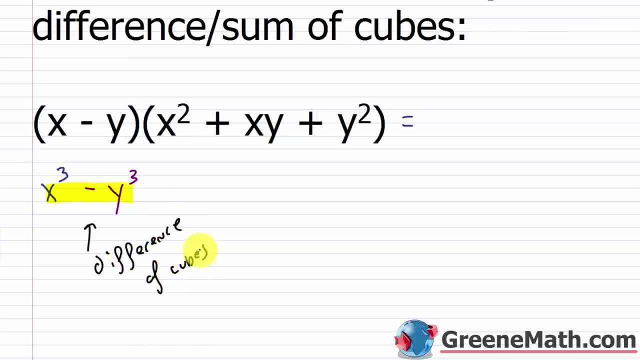 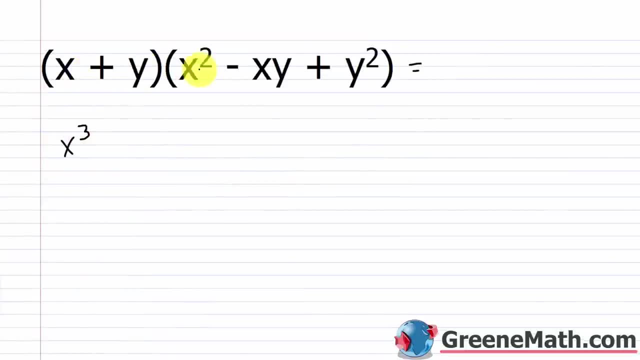 Of cubes. And we're going to look at, this one is the sum of cubes. So x times x squared is x cubed. x times minus xy is minus x squared y. x times y squared is plus xy squared. y times x squared is plus x squared y. y times negative xy is minus xy squared. y times y squared is plus y cubed. So every time you do this, you're going to get a sum of cubes. So this is the sum of cubes. 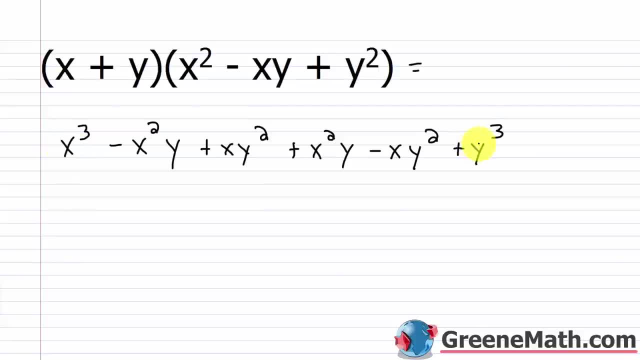 Everything's going to cancel except for the x cubed and the y cubed. So let's go ahead and do that. So negative x squared y, positive x squared y, those are going to cancel. xy squared minus xy squared, those are going to cancel. So what I'm left with is x cubed plus y cubed. So this one, 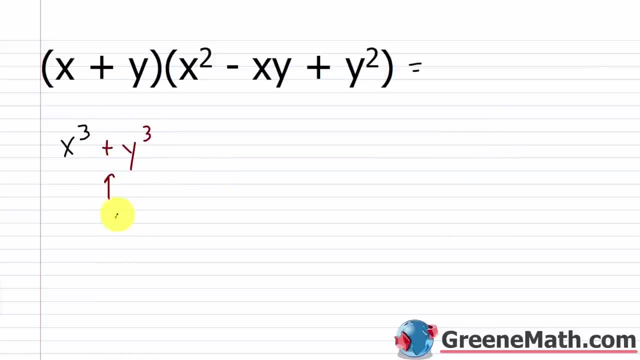 because there's an addition sign in it, is called the sum of cubes. 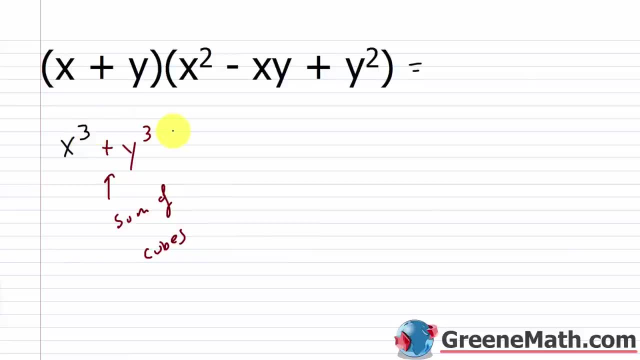 I want to erase them to the third power. It's called a cube, right? I cube it. So that's why it's called a cube. So that's why it's called a cube. So that's why it's called a cube. 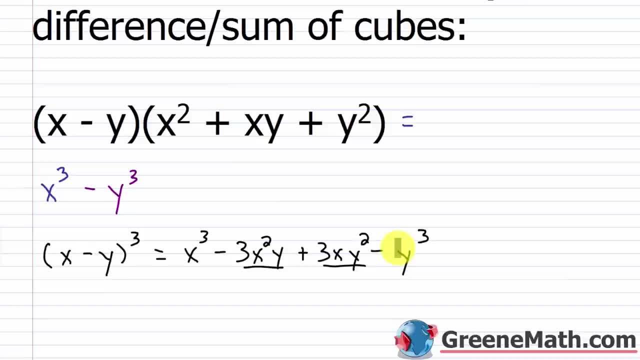 It's not the same, okay. So please understand that This formula was something we talked about when we looked at special products. So let me erase this real quick and I wanna show you the sum of cubes. So this is the difference of cubes. 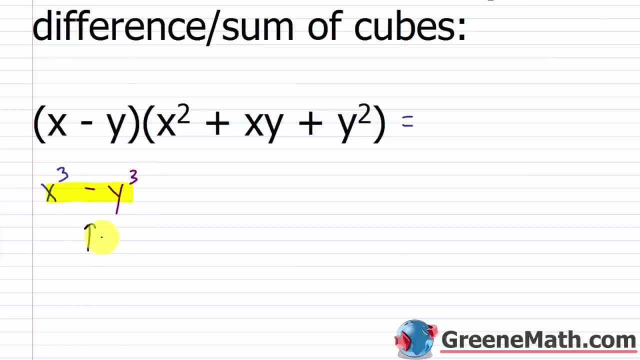 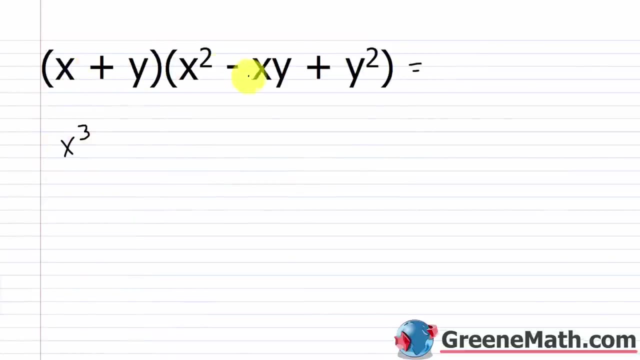 This again is the difference of cubes And we're gonna look at this one is the sum of cubes. So x times x squared is x cubed. x times minus xy is minus x squared. y, x times y squared is plus xy squared. 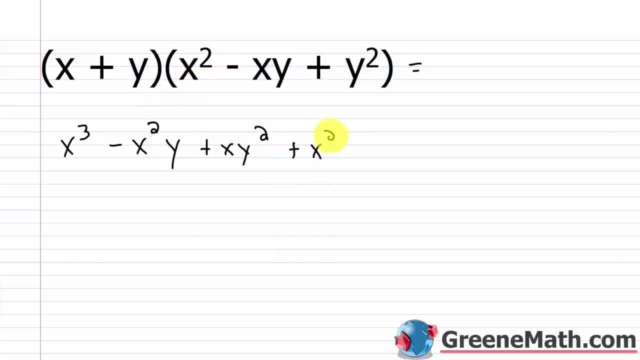 y times x squared is plus x squared. y. y times negative xy is minus xy squared. y times y squared is plus y cubed. So everything's gonna cancel except for the x cubed and the y cubed. So let's go ahead and do that. 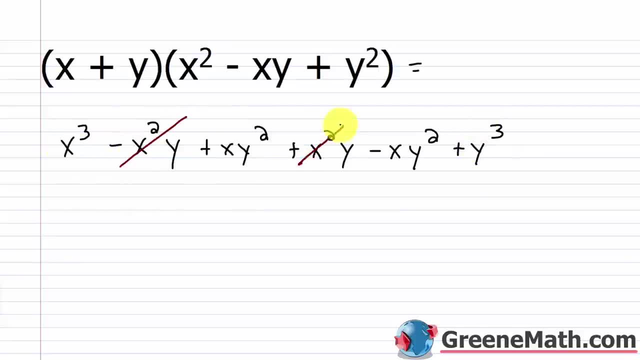 So negative x squared y, positive x squared y, those are gonna cancel. xy squared minus xy squared, those are gonna cancel. So what I'm left with is x cubed plus y cubed. So this one, because there's an addition sign in it. 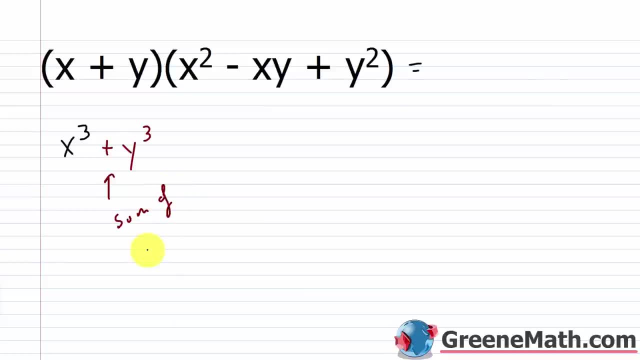 is called the sum of cubes. I wanna erase them to the third power. it's called a cube, right, I cube it. So that's why it's called the sum of cubes. You have two items there, or two terms, that are both cubed. 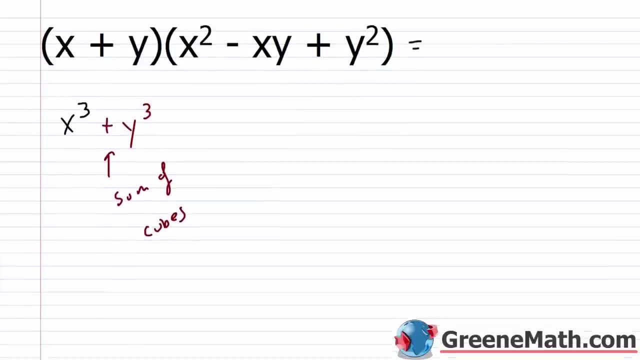 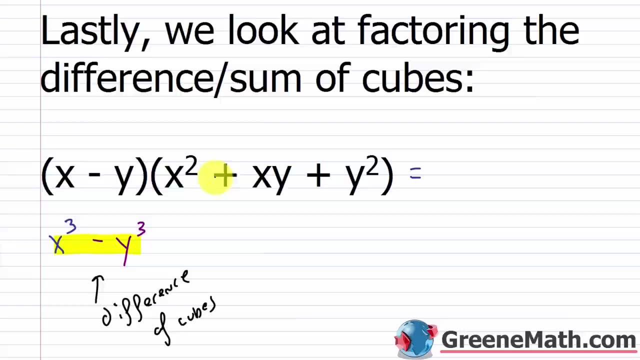 All right, so the main difference here is gonna be the sign. This is just something you have to memorize. When I have a minus, I have a minus in the first guy, and then I have all pluses in the second guy. okay, 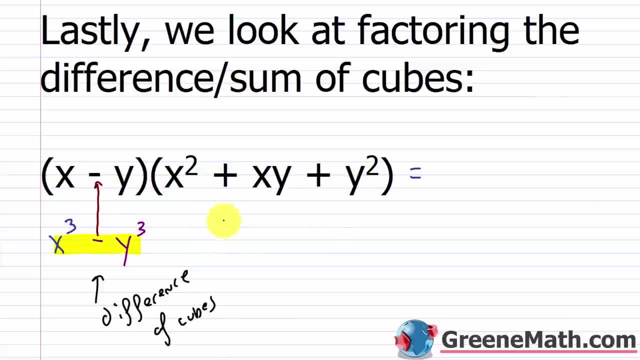 So you kinda have to remember that the first one is the same, the second one is going to be different, and then the last one is always gonna be positive, no matter what. So same, different. that's how I remember it. If you look at this, one same, different. 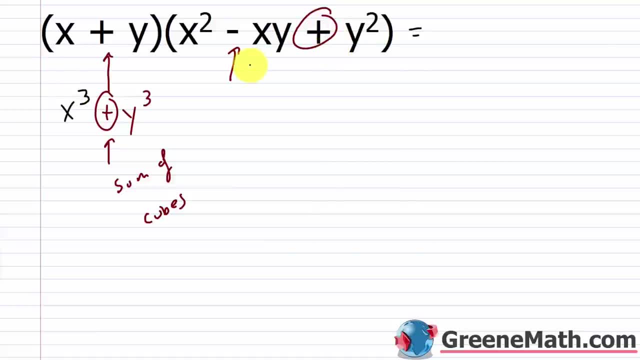 last one's always positive. okay, Same, different. that's how I remember it. You can put that on a flashcard if you want to, or maybe there's some other trick you got out there to remember it. It doesn't matter, at the end of the day, 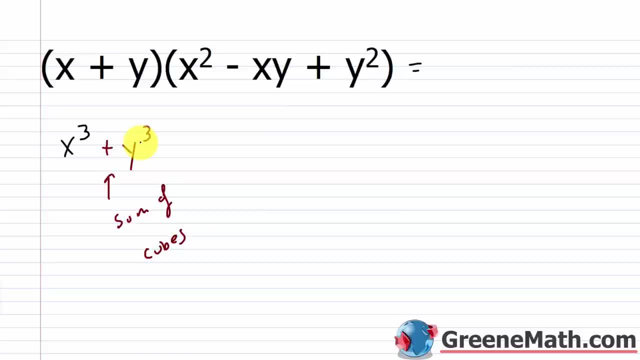 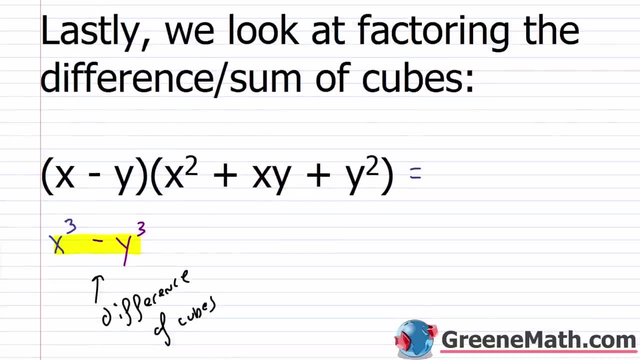 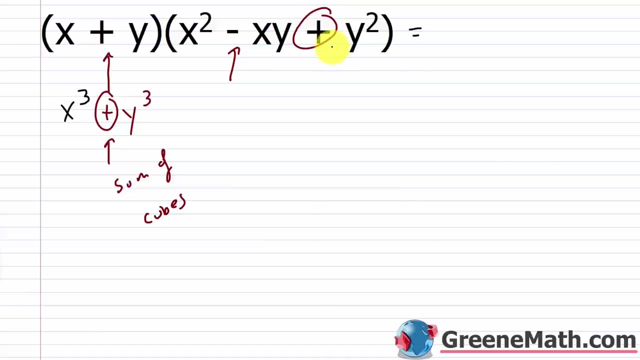 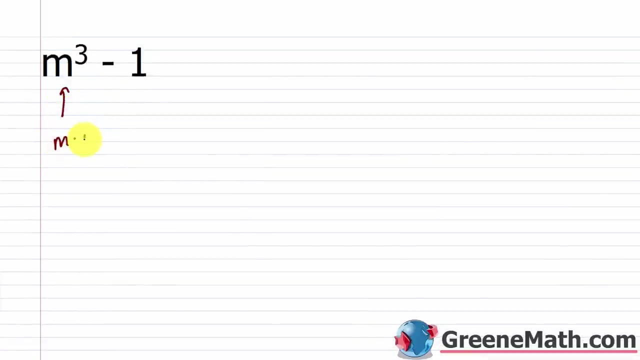 It's called the sum of cubes. You have two items there or two terms that are both cubed. All right. So the main difference here is going to be the sign. This is just something you have to memorize. When I have a minus, I have a minus in the first guy and I have all pluses in the second guy. Okay. So you kind of have to remember that the first one is the same. The second one is going to be different. And then the last one is always going to be positive no matter what. So same, different. That's how I remember it. If you look at this one, same, different. Last one's always positive. Okay. Same, different. That's how I remember it. You can put that on a flashcard if you want to. Or maybe there's some other trick you got out there to remember it. It doesn't matter at the end of the day if it's math, you know, whatever you can use to memorize it. As long as it works, it works. All right. So let's take a look at m cubed minus one. So m cubed is obviously m times m times m. What about one? Remember, one times anything is just itself. 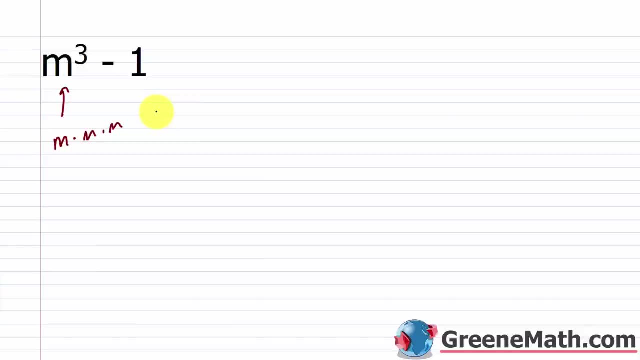 So if I have one times one, that's one. If I have one times one times one, that's still one. So this is one cubed. So this follows the format of something cubed minus something cubed. And so we can write it using that formula that we just learned. And let me rewrite that one. So if I have something that's x cubed minus y cubed, this will factor into, this is how we're going to memorize it. We have x and we have y. What's the first sign? Remember, first sign is the same. Then we have x squared and we have y squared in the end. This is always plus. What's the sign here? Remember, same, different. So this is minus, this will be plus, and then you have xy. So following this formula, all I need to do is think about, okay, this is what's cubed and this is what's cubed. So in the first thing that's cubed, it's going to go where? 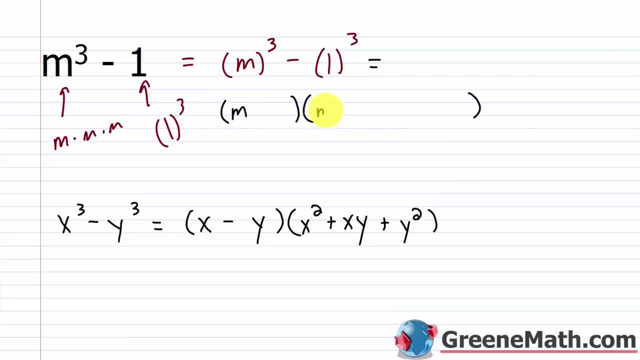 It's got a position here. It's got a position here that's squared. And then it's got a position here. 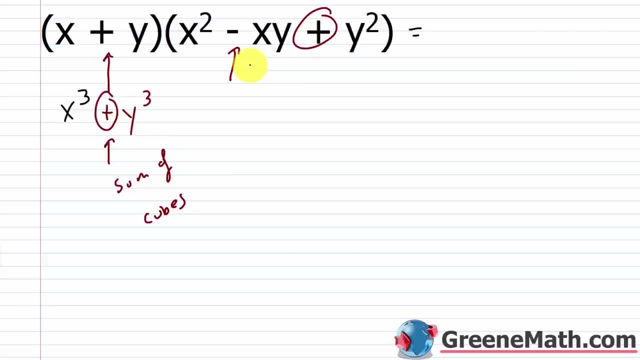 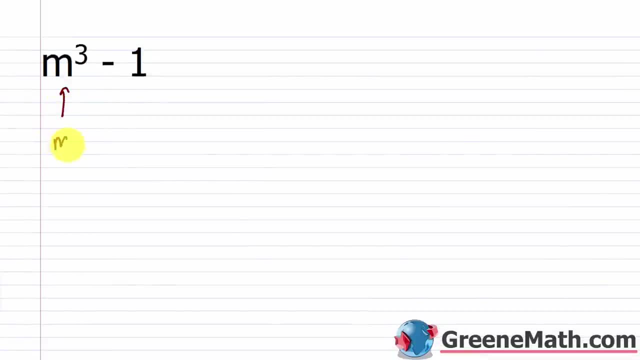 if it's math, you know. whatever you can use to memorize it, as long as it works, it works All right. so let's take a look at m cubed minus one. So m cubed is obviously m times m times m. 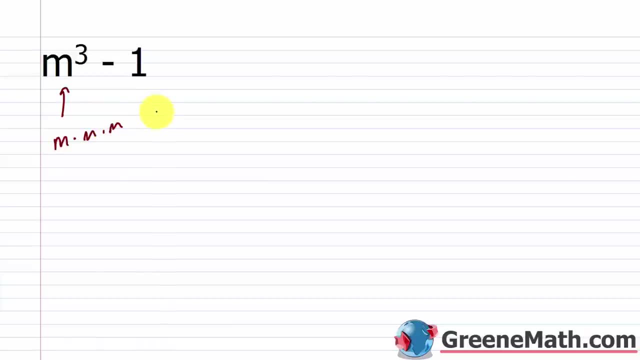 What about one Remember? one times, anything is just itself. So if I have one times one, that's one. If I have one times one times one, that's still one. So this is one cubed. So this follows the format of one cubed. 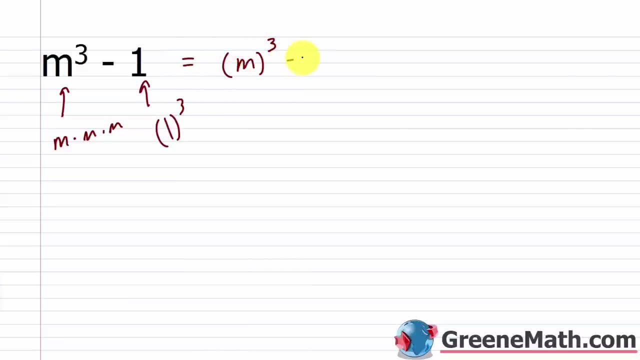 So this follows the format of one cubed, So this follows the format of something cubed minus something cubed, And so we can write it using that formula that we just learned. And let me rewrite that one, So if I have something that's x cubed minus y cubed, 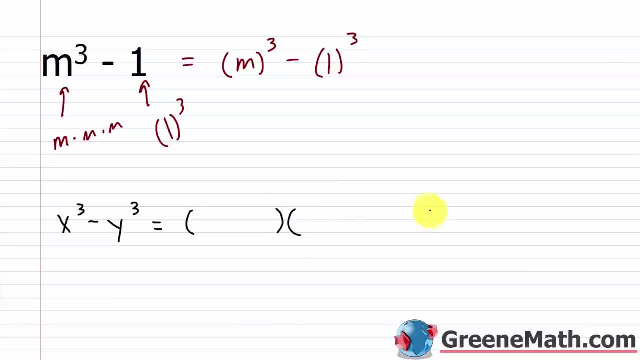 this will factor into. this is how we're gonna memorize it. We have x and we have y. What's the first sign? Remember? first sign is the same. Then we have x squared and we have y squared in the end. 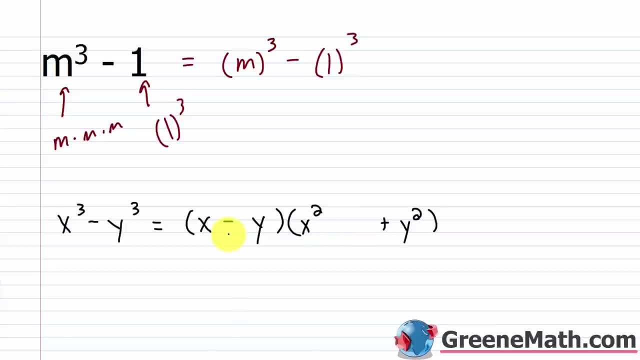 This is always plus. What's the sign here? Remember, same, different. So this is minus, this will be plus, and then you have xy. So, following this formula, here, all I need to do is think about: okay, this is what's cubed and this is what's cubed. 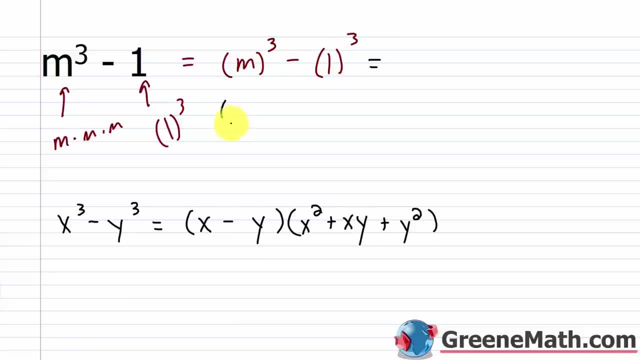 So, in the first thing, that's cubed, it's gonna go where. It's got a position here, It's got a position here, that's squared, And then it's got a position here, And then that's it. We're gonna subtract this guy. 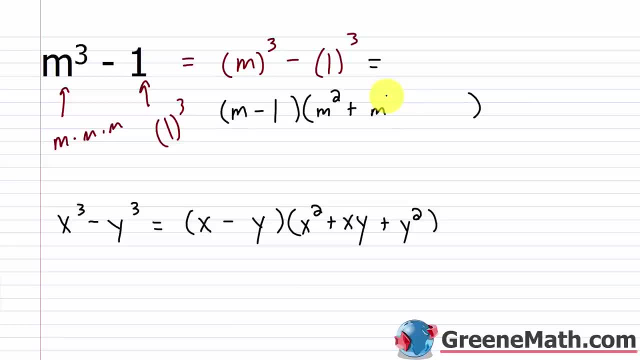 Then we're going to add one times this guy, which is just itself, And then we're gonna add that guy squared, which is just one. So we get the quantity m minus one times the quantity m squared plus m plus one. And I know these are a lot more challenging. 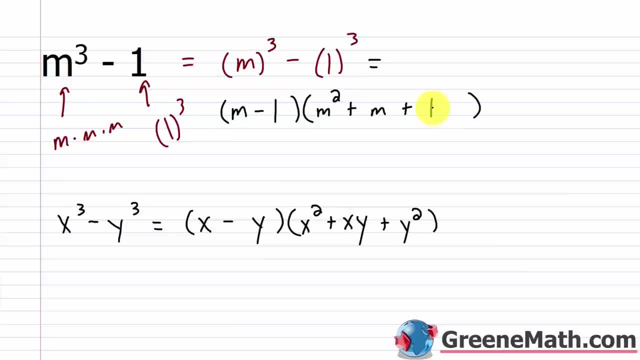 especially when you see them. at first It's like, hey, how am I gonna remember that If you do enough practice with this? I suggest doing a lot, a lot of practice, because by the time you get to algebra two, you're going to need this formula. 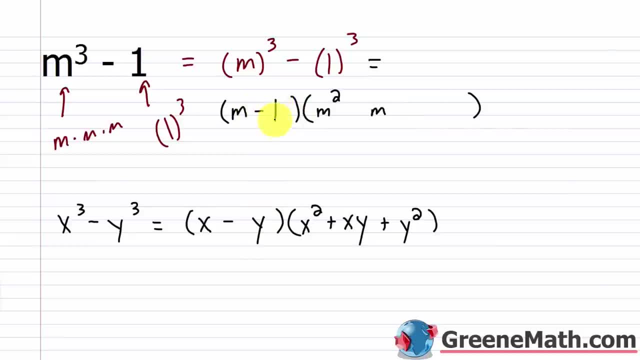 And then that's it. We're going to subtract this guy. Then we're going to add one times this guy, which is just itself. And then we're going to add that guy squared, just one. So we get the quantity m minus one times the quantity m squared plus m plus one. 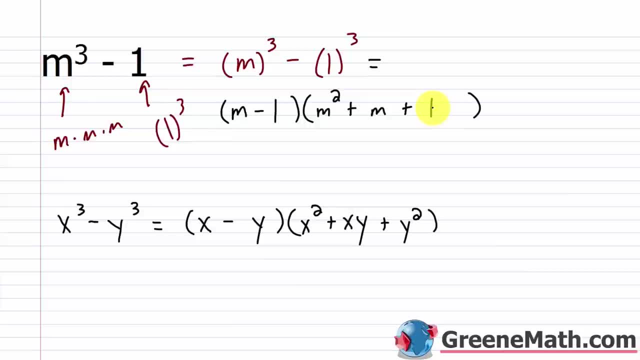 And I know these are a lot more challenging, especially when you see them at first. It's like, hey, how am I going to remember that? If you do enough practice with this, I suggest doing a lot, a lot of practice because by the time you get to algebra two, you're going to need this formula to get through a lot of the tests that you're going to take, especially like the SAT and the ACT, all these standardized tests that you're going to take where time matters, right? So if you know it's worth taking these test I think you can go through and crank these things out very, very 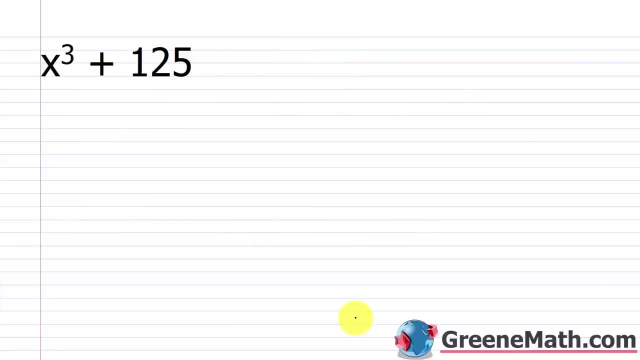 quickly and be assured that you have the right answer. All right. So let's look at x cubed plus 125. So what's our formula? Again, x cubed plus y cubed. So the first sign is the 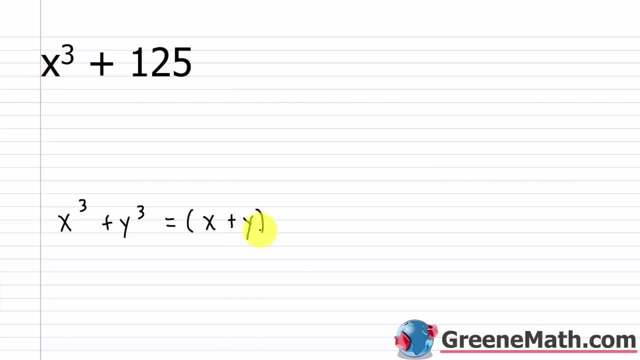 same. So we have a plus there, so this is going to be x plus y, very easy to remember. Then the next one, you have x squared, the sign that comes after that is different. This is plus, so this is going to be minus, then it's x y, and then it's plus, this one's always plus, and then it's also x. 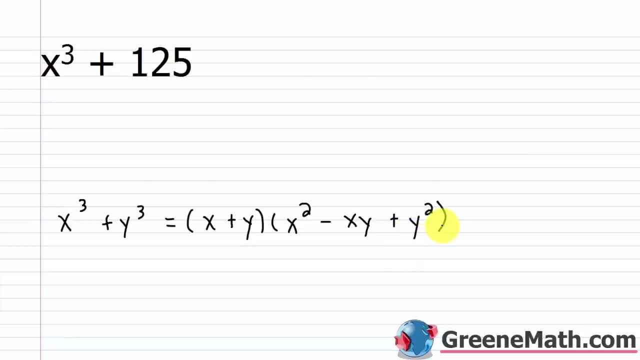 y squared. Okay so very very easy to remember. So kind of following this format if I look at this I have x cubed and I have 125. So 125 is 5 cubed. So all I need to do is put what? It's going to be x plus 5. x is what's cubed here. 5 is what's cubed here. So we have x plus y here. x is what's cubed. 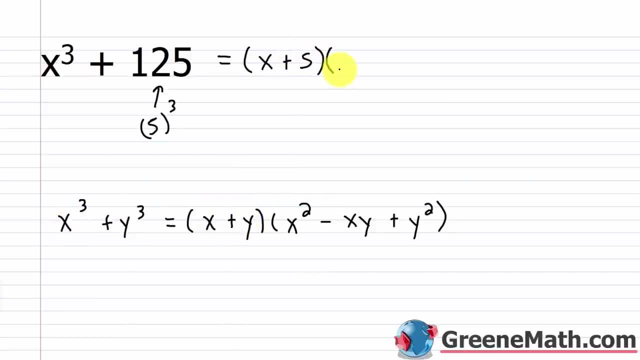 y is what's cubed. So we have x plus y. Here we have x plus 5. Then following this format we have x squared. So we have x squared minus xy. In this case we have x times 5. So 5x. And then plus we have y squared here. So whatever is cubed that's now going to be squared. So 5 is what's cubed. So that's going to be squared. 5 squared is 25. So we get the quantity x plus 5 times the quantity x squared minus 5x plus 25. Let's take a look at one final problem. So what is x cubed? 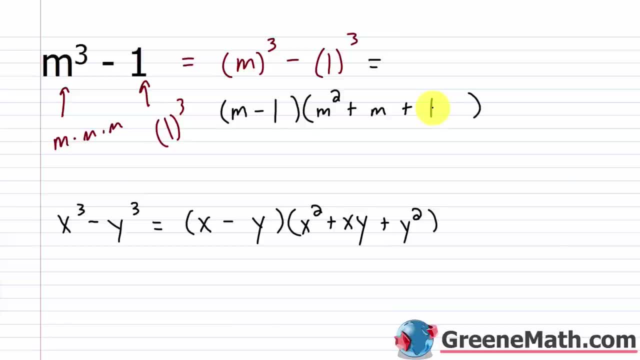 to get through a lot of the tests that you're gonna take, especially like the SAT and the ACT, all these standardized tests that you're gonna take where time matters, right. So if you know the formulas, you can go through and crank these things out. 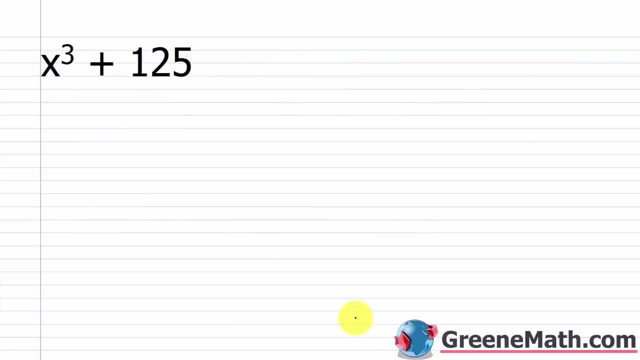 very, very quickly and be assured that you have the right answer. All right, so let's look at x cubed plus 125.. So what's our formula Again? x cubed plus y cubed. So the first sign is the same. 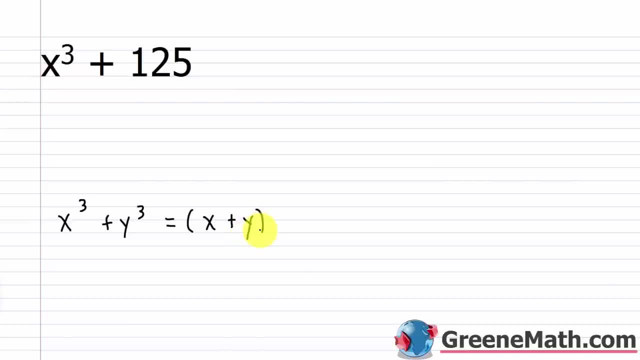 So we have a plus there. So this is gonna be x plus y. Very easy to remember. Next one: you have x squared. The sign that comes after that is different. This is plus, so this is gonna be minus, Then it's xy and then it's plus. 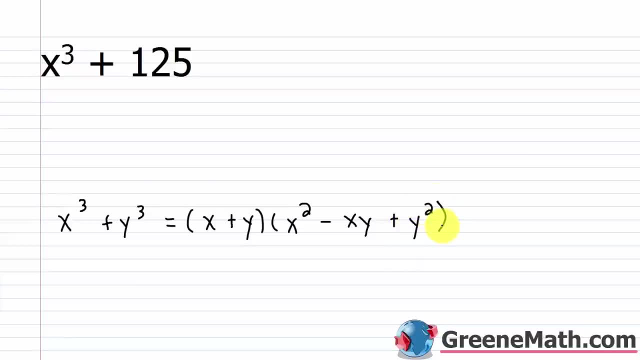 This one's always plus, and then it's y squared, Okay, so very, very easy to remember. So, kind of following this format, if I look at this, I have x cubed and I have 125.. So 125 is five cubed. 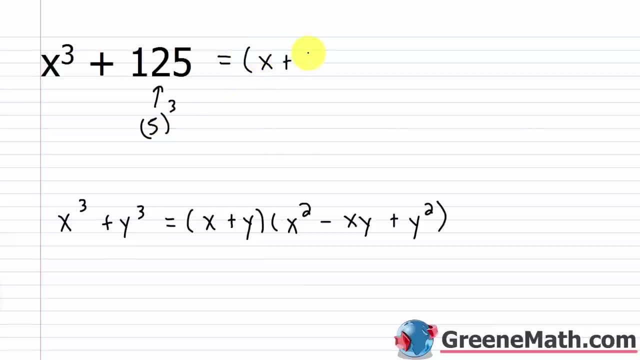 So all I need to do is put what It's gonna be: x plus five. X is what's cubed Here, five is what's cubed here. So we have x plus y here. X is what's cubed, Y is what's cubed. 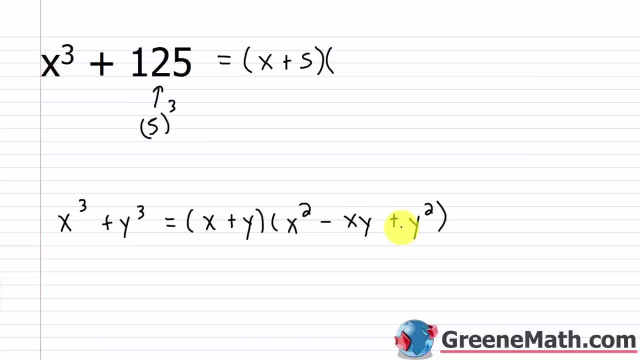 So we have x plus y. Here we have x plus five. Then, following this format, we have x squared, So we have x squared minus xy. In this case we have x times five, so five x, And then plus we have y squared here. 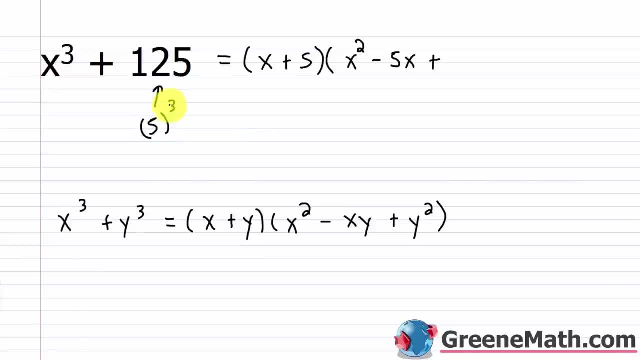 So whatever is cubed, that's now gonna be squared. So five is what's cubed, so that's gonna be squared. Five squared is 25.. So we get the quantity x plus five times the quantity x squared minus five x plus 25.. 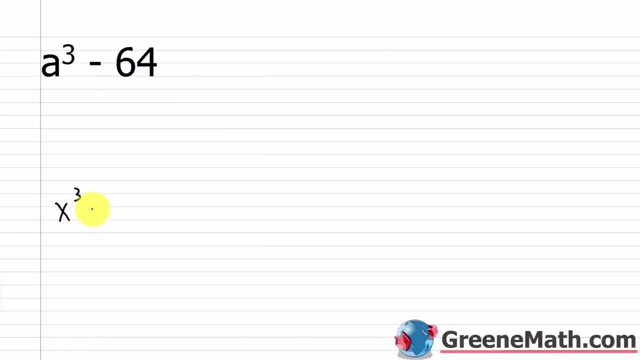 All right, let's take a look at one final problem. So what is x cubed? again minus y cubed. So again, the first sign is the same. So x minus y- same sign. Then the next one that we're gonna think about. 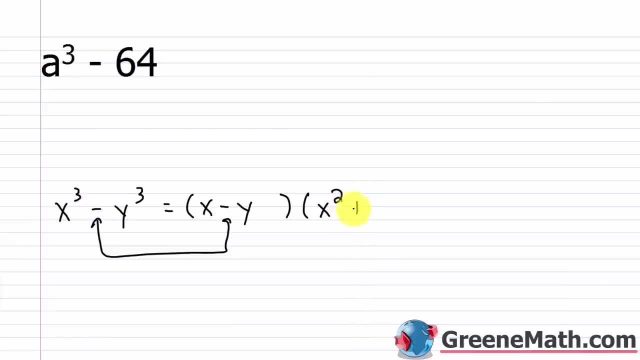 after the x squared is different. So this is a minus. so now it's gonna be a plus, And then we would have xy, And then this sign right here: this is always a plus, So we have plus, and then we have y squared. 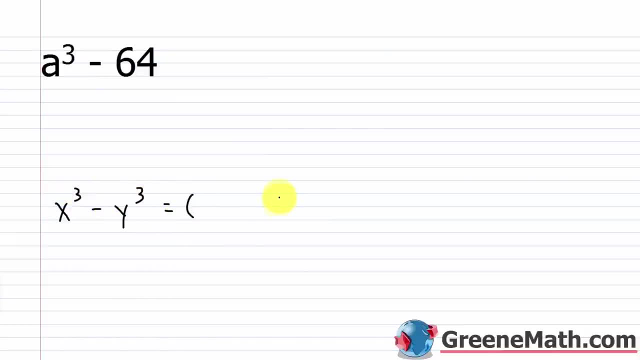 Again minus y cubed. So again the first sign is the same. So x minus y. Same sign. 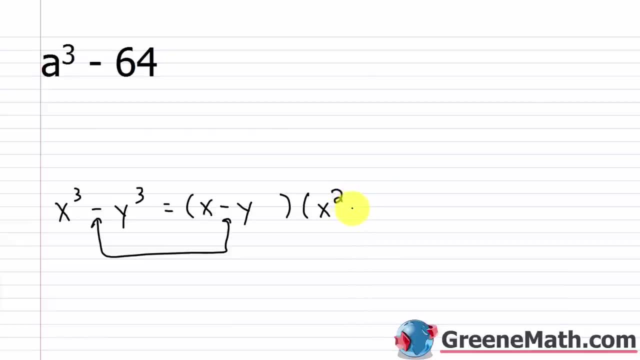 Then the next one that we're going to think about after the x squared is different. So this is a minus. So now it's going to be a plus. And then we would have xy. And then this sign right here is always a plus. So we have plus. And then we have y squared. So following this format we have a cubed. A is what's cubed. 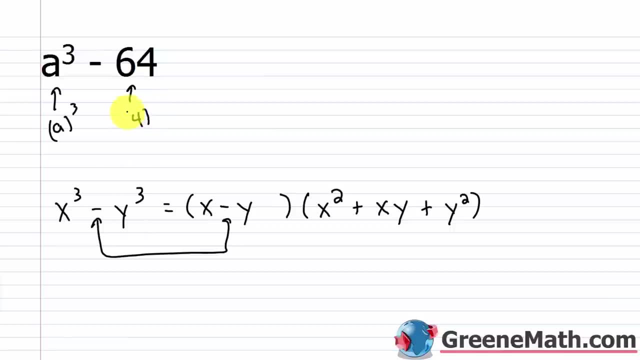 We have 64. 64 is 4 cubed. So 4 is what's being cubed. So follow the format. So whatever's being cubed in the first position. In this case that's a minus whatever's being cubed in the second position. In this case that's 4. Then times. Whatever's being cubed in the first position is now squared. So that's a squared. Then plus. We have whatever's cubed in the first position times whatever's cubed in the second position. So a times 4 or 4a. Then plus. 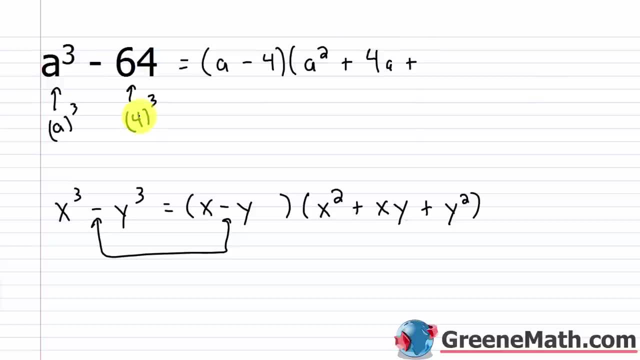 Whatever's cubed in the last position. In this case that's a 4. We're going to square. Just like it is here. So 4 squared is 16. Close the parentheses and we have the quantity a minus 4 times the quantity a squared plus 4a plus 16. So just something to keep in mind. These formulas are going to greatly speed up your homework and your tests. So something you definitely want to memorize. What I always suggest for my tutoring students is write out the formula that you know and then just make the comparison. Like we're doing here. Okay if I know x cubed minus y cubed is the quantity x minus y times the quantity x squared plus xy plus y squared. I can just represent everything and then go through and match up my formula and do it like that for a while. And you know 20 or 25 problems later you won't even need to write the formula down. You'll have this stuff memorized. Hello and welcome to 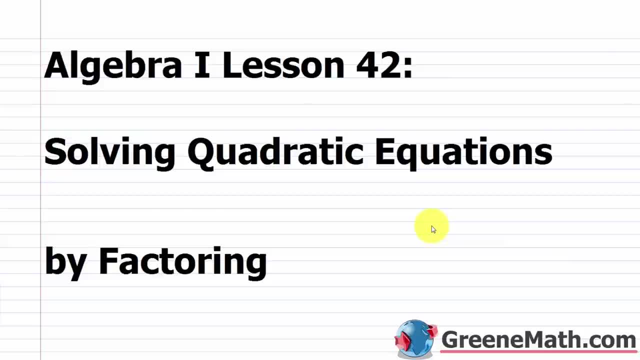 Algebra 1 Lesson 42. In this video we're going to learn about solving quadratic equations by factoring. So a quadratic equation is a formula that you can use to solve a quadratic equation. 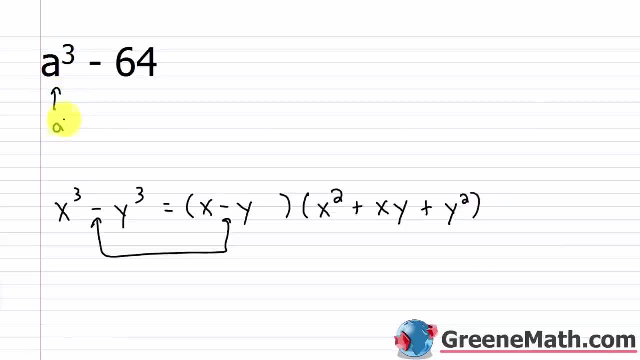 So, following this format, we have a cubed, A is what's cubed, and we have 64.. 64 is four cubed, so four is what's being cubed. So follow the format. So whatever's being cubed in the first position. 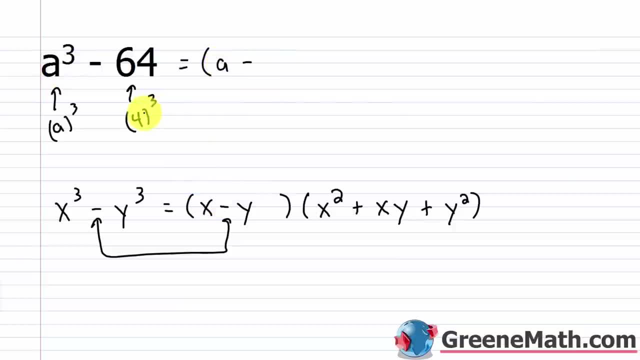 in this case that's a minus. whatever's being cubed in the second position- in this case that's four, Then times: Whatever's being cubed in the first position is now squared, so that's a squared, Then plus. 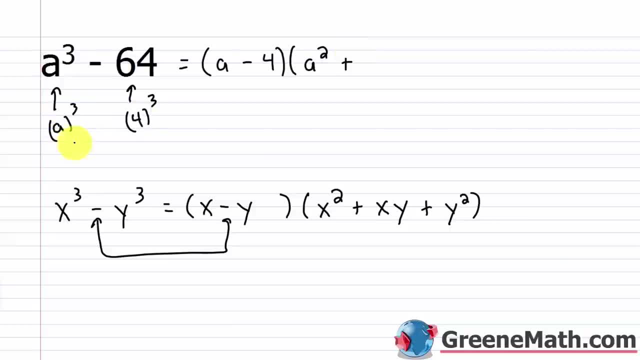 We have whatever's cubed in the first position times whatever's cubed in the second position. So a times four or 4a, Then plus Whatever's cubed in the last position. in this case that's a four. 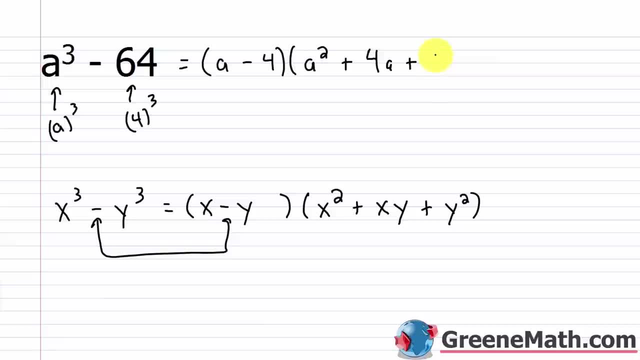 We're going to square just like it is here. So four squared is 16.. Close the parentheses and we have the quantity a minus four times the quantity a squared plus 4a plus 16.. So just something to keep in mind. 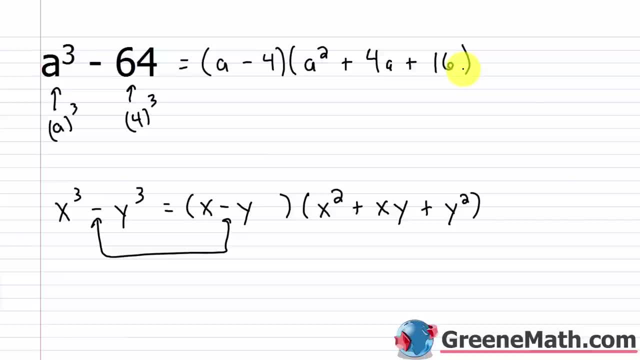 These formulas are gonna greatly speed up Your homework and your tests, So something you definitely want to memorize. What I always suggest for my tutoring students is write out the formula that you know and then just make the comparisons, like we're doing here. 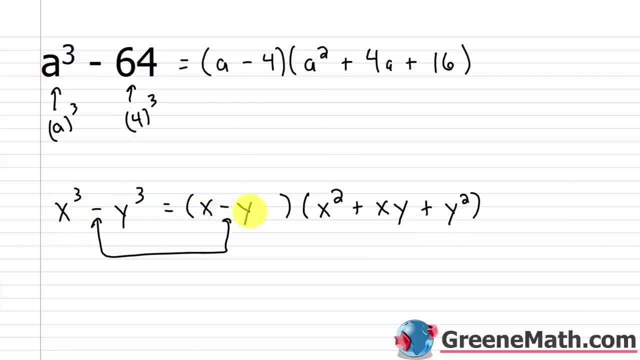 Okay, if I know, x cubed minus y cubed is the quantity x minus y times the quantity x squared plus xy plus y squared. I can just represent everything and then go through and match up my formula and do it like that for a while. 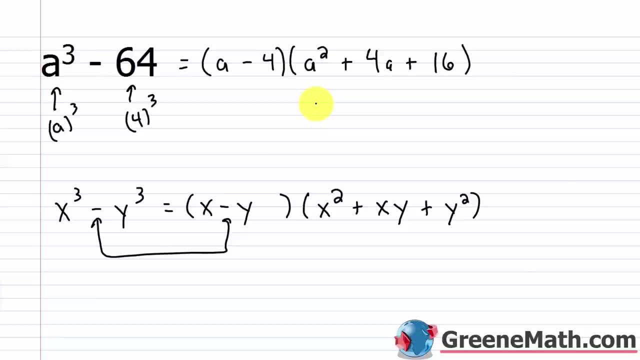 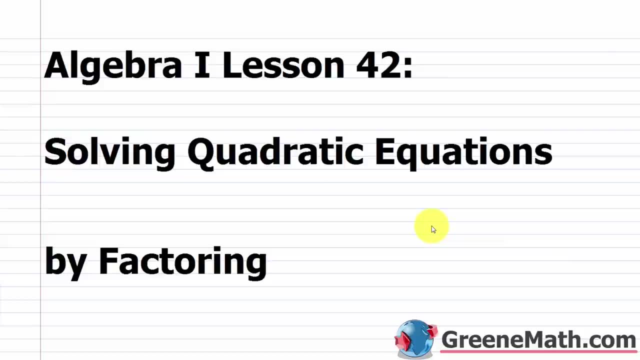 and you know 20 or 25 problems later. you won't even need to write the formula down. you'll have this stuff memorized. Hello and welcome to Algebra 1, Lesson 42.. In this video, we're gonna learn about 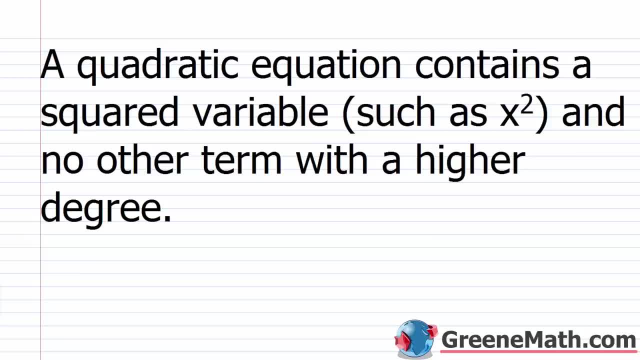 solving quadratic equations by factoring. So a quadratic equation contains a squared variable. So I have here, such as x squared, or it could be y squared, or z squared, or whatever variable you've chosen to work with in that equation- squared. And then I have here and no other term with a higher degree. 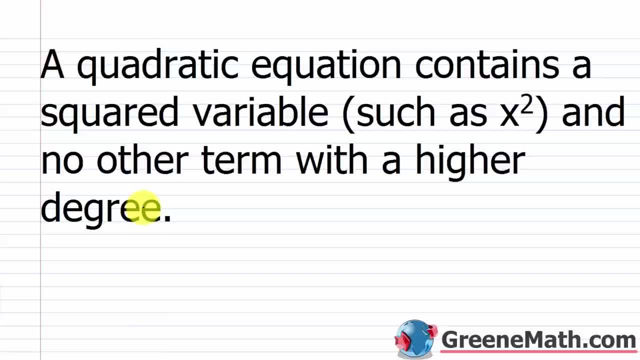 So in other words, the largest thing that you're gonna have on your variable is going to be a two right. You can't have x cubed or x to the sixth power. That's not gonna be involved in a quadratic equation. So generally we think about quadratic equations. 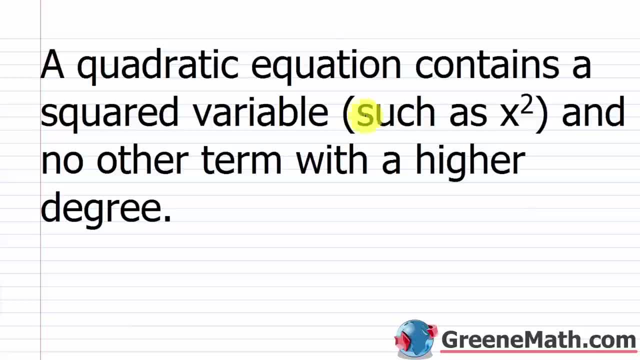 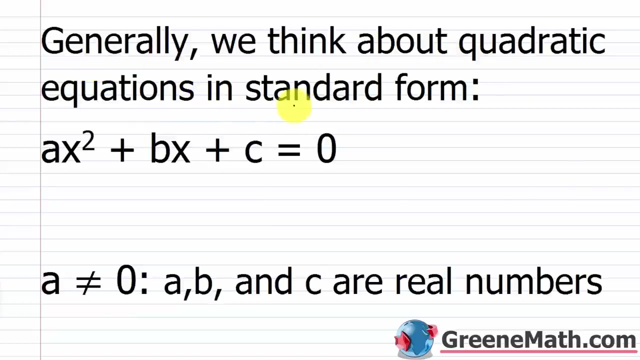 It contains a squared variable. So I have here such as x squared or it could be y squared or z squared or whatever variable you've chosen to work with in that equation squared. And then I have here and no other term with a higher degree. So in other words the largest exponent that you're going to have on your variable is going to be a 2. Right you can't have x cubed or x to the 6th power. That's not going to be involved in a quadratic equation. So generally we think about quadratic equations in standard form. So we have ax squared plus bx plus c and then because it's an 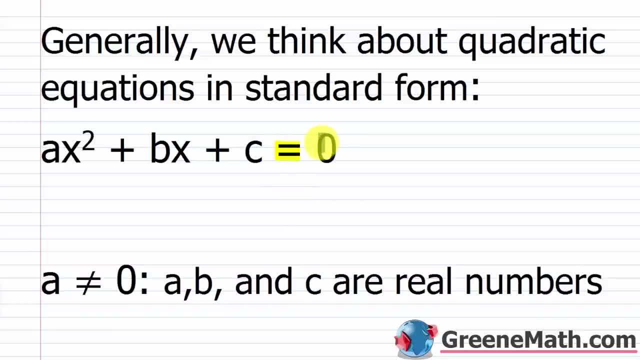 equation we have the equal sign and we set it equal to 0. Okay so it's set equal to 0. Now remember that a is the coefficient for the x squared term. So this is a coefficient. B is the coefficient for 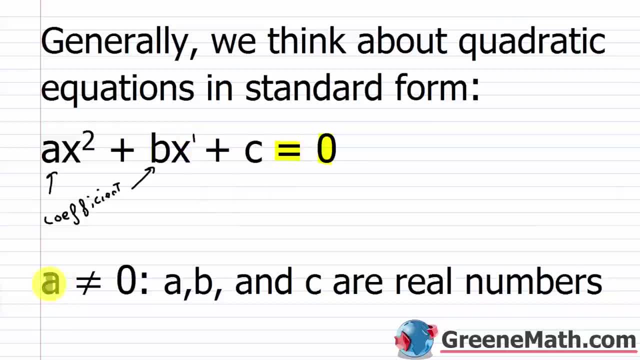 that. So if we look here we have one restriction. So a cannot be equal to 0. And why do you think that is. Well again this is the coefficient for the x squared term. And for us to have a quadratic equation we've got to have a variable that is squared in that equation. Right that's part of the definition. So we have ax squared plus bx plus c equals 0 where a is not equal to 0. And then a b 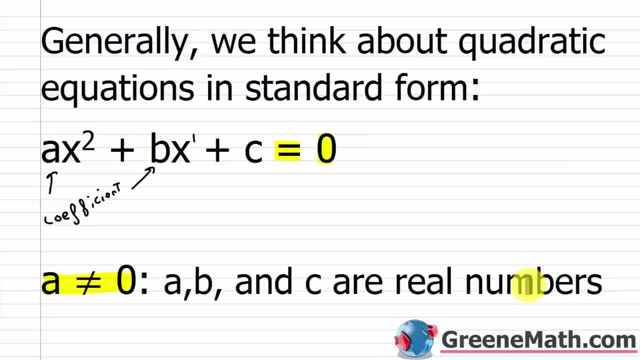 and c are real numbers. And I know I haven't given you an official definition for that yet. 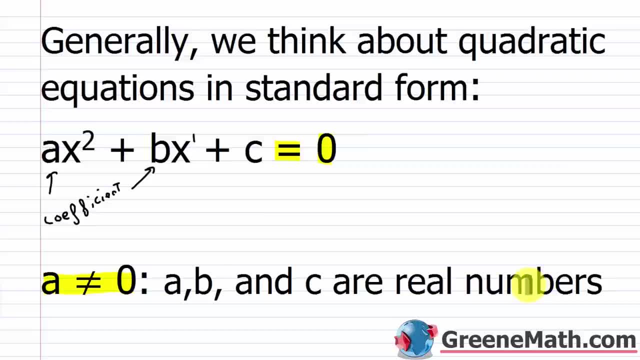 But it's just any kind of number that you can think of at this point. So here are some examples. 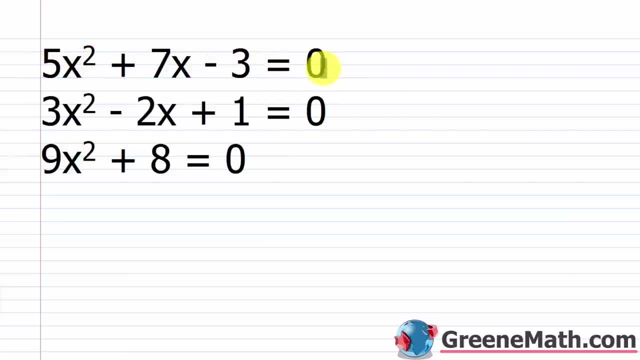 We have 5x squared plus 7x minus 3 and this equals 0. We have 3x squared minus 2x plus 1 equals 0. We have 9x squared plus 8 equals 0. Now you might see these two up here and say well those those kind of fit the format of you know ax squared plus bx plus c. Right where a in this case is equal to 0. And then we have bx squared plus bx plus c. Right where a in this case is 5. B here is 7 and c is negative 3. And then in this case a is 3. B is negative 2 and c is 1. But 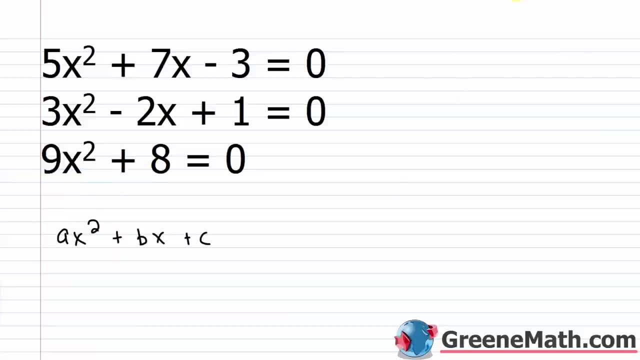 what about this one where we have 9x squared plus 8 equals 0. It looks like I'm missing this bx term. 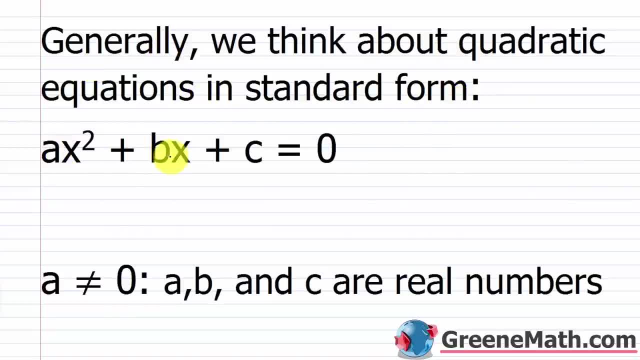 in standard form. So we have ax squared plus bx plus c, and then, because it's an equation, we have the equal sign and we set it equal to zero. Okay, so it's set equal to zero. Now, remember that a is the coefficient for the x squared. 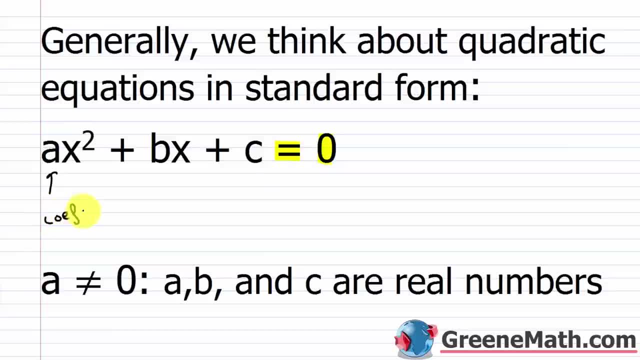 and b is the coefficient for the x to the first power term, And then c is a constant. So if we look here, we have one restriction. So a cannot be equal to zero. And why do you think that is? Well, again, this is the coefficient. 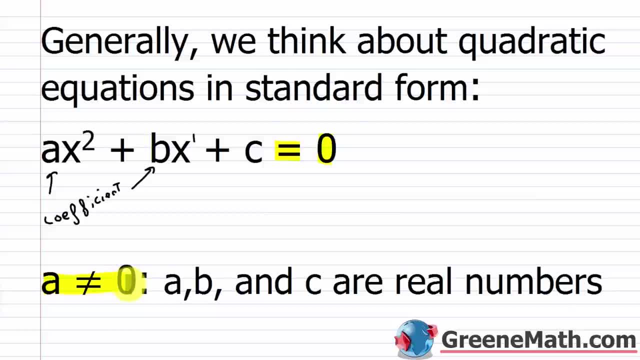 for the x squared term And for us to have a quadratic equation, we've gotta have a variable that is squared in that equation, right? That's part of the definition. So we're gonna have a variable that is squared in that equation, right? 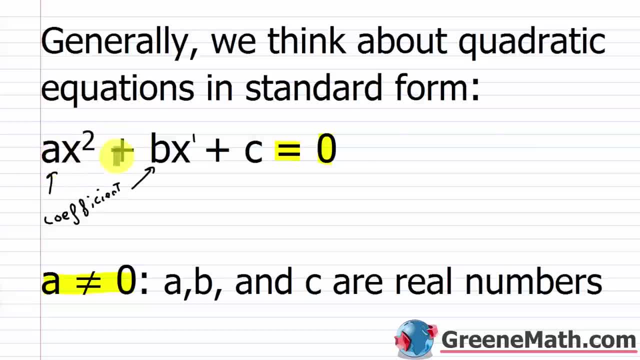 That's part of the definition. So we have ax squared plus bx plus c equals zero, where a is not equal to zero. and then a, b and c are real numbers And I know I haven't given you an official definition for that yet. 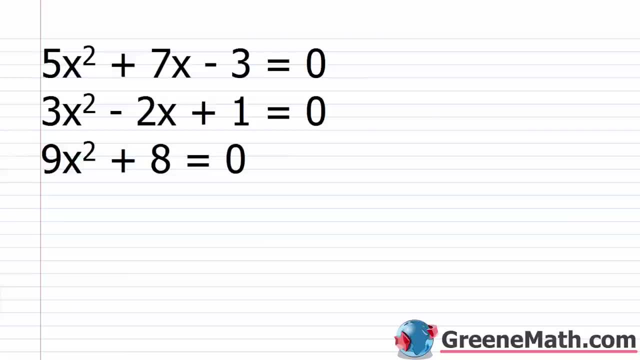 but it's just any kind of number that you can think of at this point. So here are some examples. We have five x squared plus seven x minus three, and this equals zero. We have three x squared minus two x plus one equals zero. 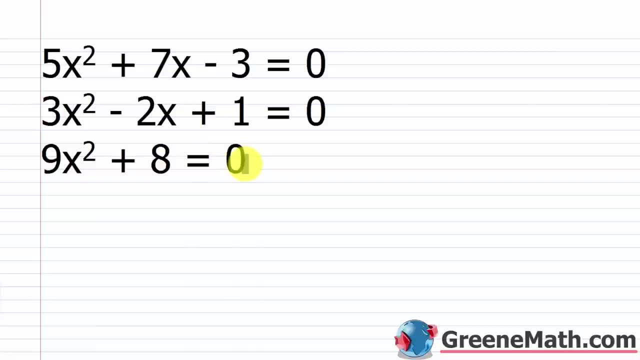 We have nine x squared plus eight equals zero. We have three x squared minus two x plus one equals zero. We have nine x squared plus eight equals zero. Now you might see these two up here and say, well, those kind of fit the format. 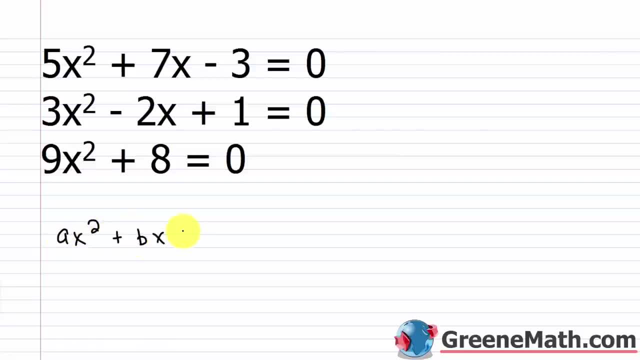 of ax squared plus bx plus c, right, Where a in this case is five, b here is seven and c is negative three. And then, in this case, a is three, b is negative two and c is one. But what about this one? 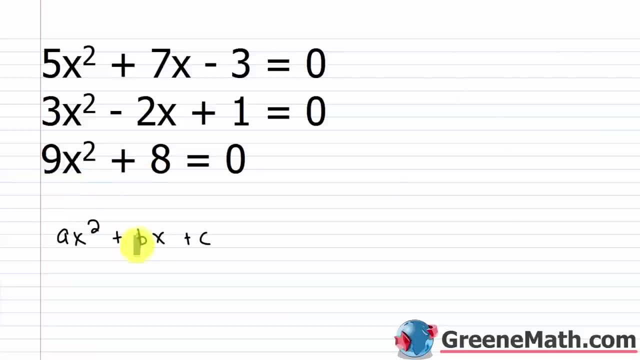 where we have nine x squared plus eight equals zero. It looks like I'm missing this bx term. right, I'm missing that, But remember we defined b as being able to be any real number, So that means b could be zero. 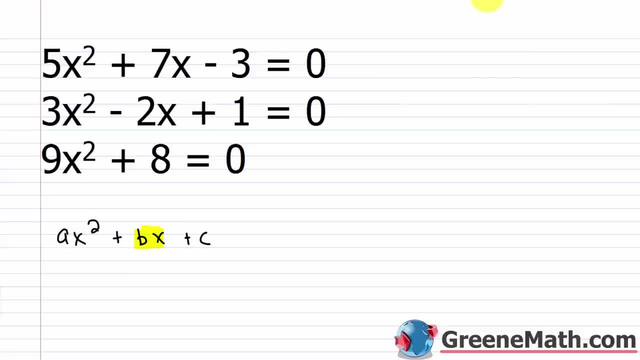 Right I'm missing that. But remember we defined b as being able to be any real number. So that means b could be 0. And remember if you multiply something by 0 it becomes 0. So it would just disappear. So 9x squared plus we could put 0. And then we have 9x squared plus 8 equals 0. And then we have 9x squared plus we could put 0. And then we would just disappear. So if I put since we have basically aех why 3x squared plus 8 equals 0 neighbor into a common denominator of 0x 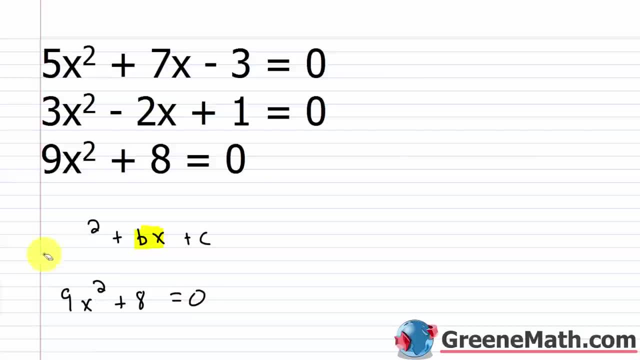 plus 8 equals 0. 0 times x is 0. So if I put plus 0 I can just get rid of it and plug that into there. So here we have 8 plus x square root 2 plus 2x squared plus 6x squared plus 4x squared 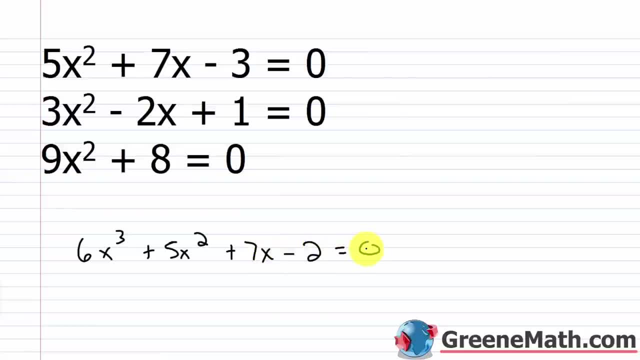 minus 3x square root of x squared plus 6x squared 2 times x to zero. And so we can pet that area into our 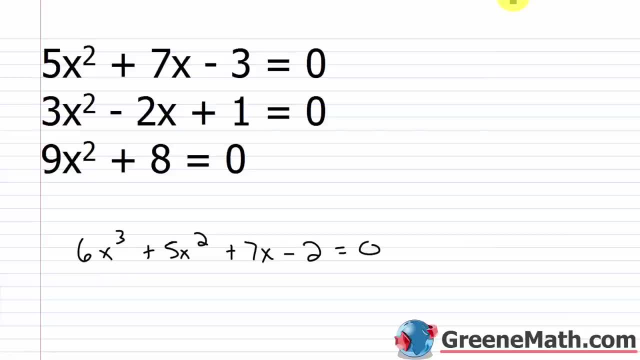 Remember, the highest exponent on your variable is going to be a two with a quadratic equation. This one has a three here. So that's not going to be a quadratic equation. 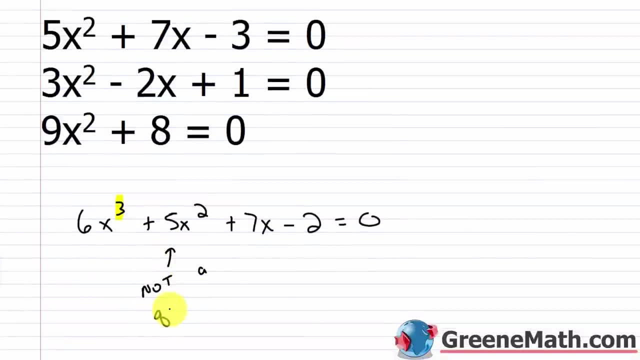 So this is not a quadratic equation. 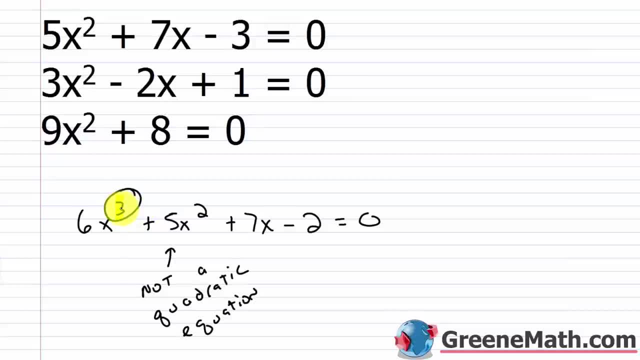 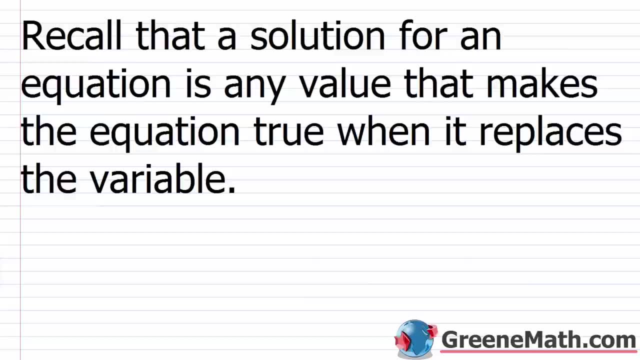 And again, that's specifically because you have an x cubed there. So pretty easy overall, when we think about the definition of a quadratic equation, and just think about when we say we're writing it in standard form, think back to the standard form of a polynomial, right, if I have, you know, ax squared, plus bx plus C, when we think about this trinomial here, it's written in standard form, because the exponents go in descending order, I start with the highest, which is a two, then I go to a one, and then 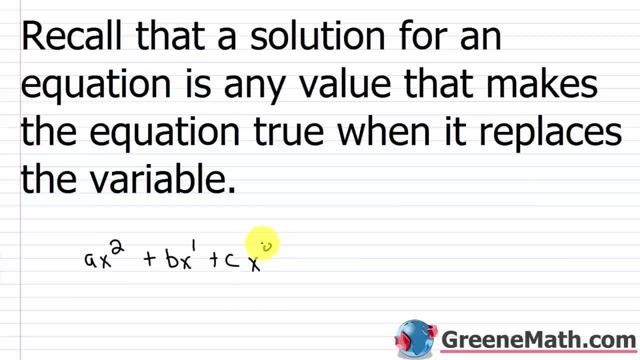 I go kind of to where I don't have a variable, where I could say this is x to the power of zero if I wanted to. 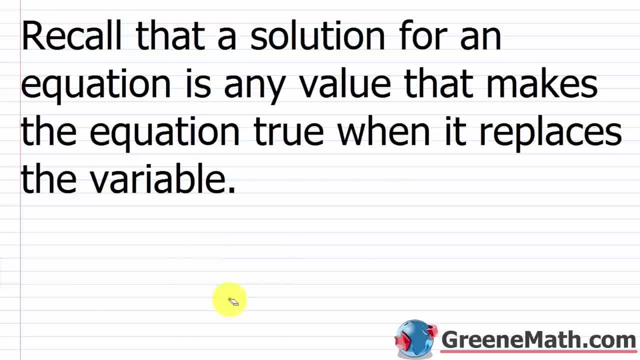 So that's how standard form is for a quadratic equation as well. Just remember that. And it'll make it easy for you to write it out each time. 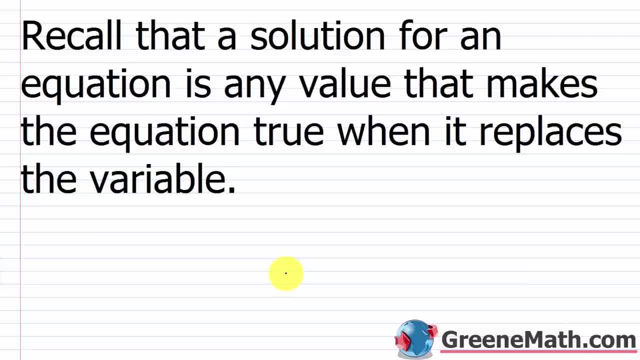 Now let's kind of move into the main part of the lesson, we're going to start solving these quadratic equations using factoring. 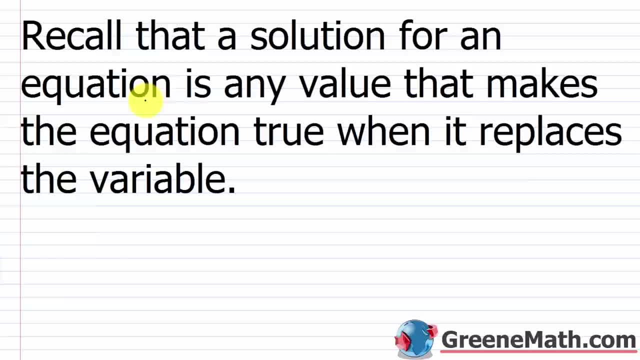 So I want you to first recall that a solution for an equation is any value or could be values that makes the equation true when it replaces the variable, or it could be variables if you have more than one. 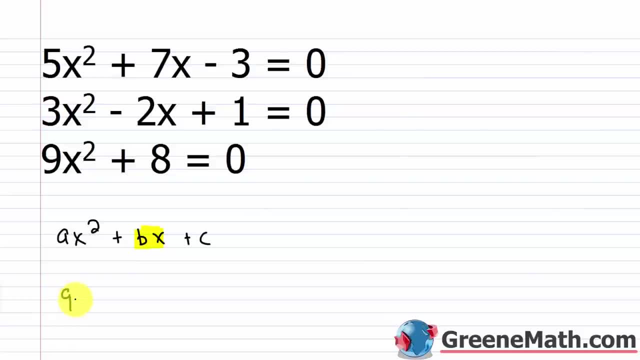 And remember, if you multiply something by zero, it becomes zero, so it would just disappear. So nine x squared plus, we could put zero. x plus eight equals zero. Zero times x is zero. so if I put plus zero, I can just get rid of it and simplify this. 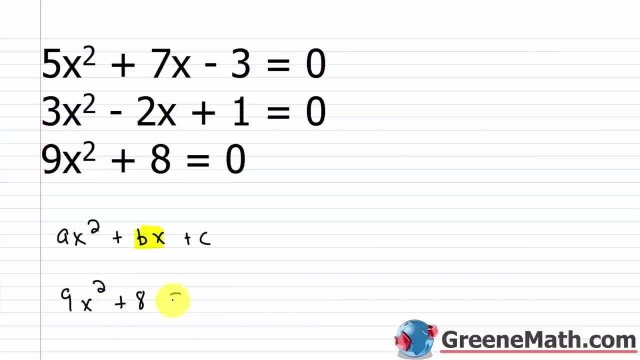 and put: plus eight equals zero. Now they might throw something at you on a test and say: is something like I don't know. let's say six x cubed plus five x squared, plus seven x minus two equals zero. is that a quadratic equation? 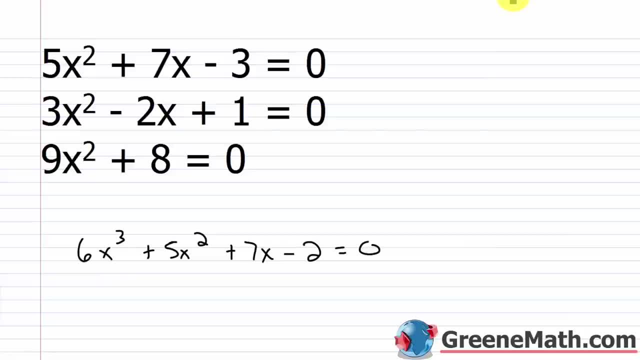 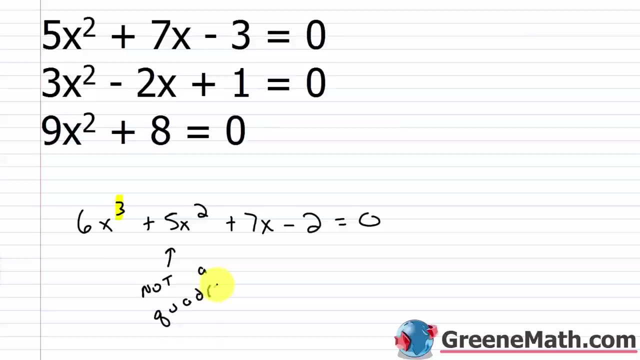 The answer is no. Remember, the highest exponent on your variable is going to be a two with a quadratic equation, This one has a three here, So that's not gonna be a quadratic equation. So this is not a quadratic. I'll put equation. 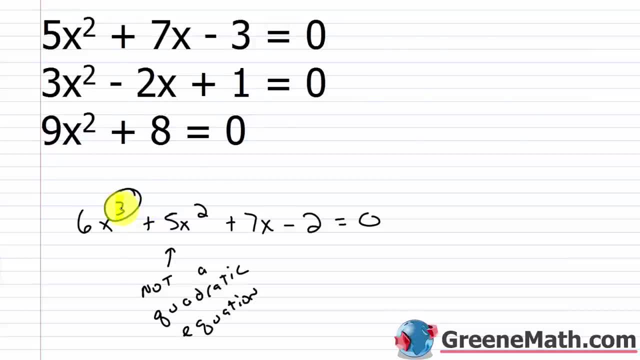 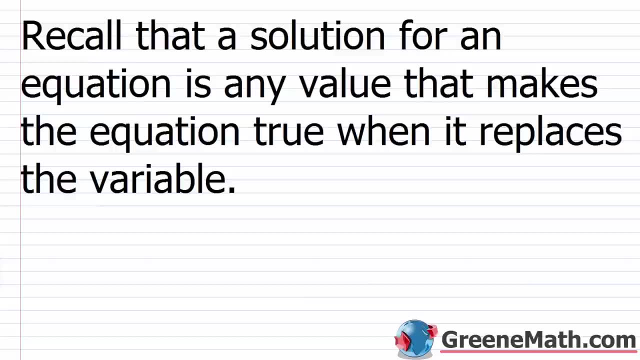 And again, that's specifically because you have an x cubed there, So pretty easy overall. when we think about the definition of a quadratic equation, And just think about when we say we're writing it in standard form, think back to the standard form. 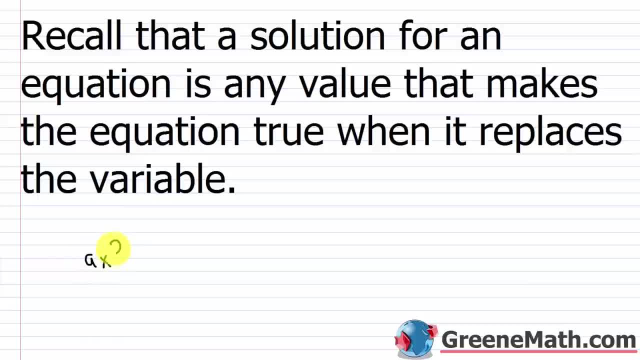 of a polynomial right If I have ax squared plus bx plus c. when we think about this trinomial here. it's written in standard form because the exponents go in descending order. I start with the highest, which is a two. 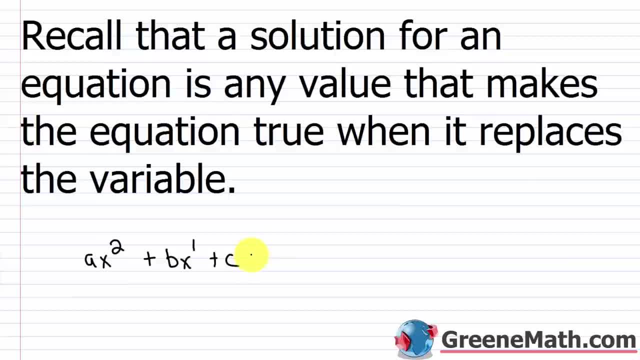 then I go to a one and then I go kinda to where I don't have a variable, where I could say: this is x to the power of zero if I wanted to. So that's how standard form is for a quadratic equation as well. 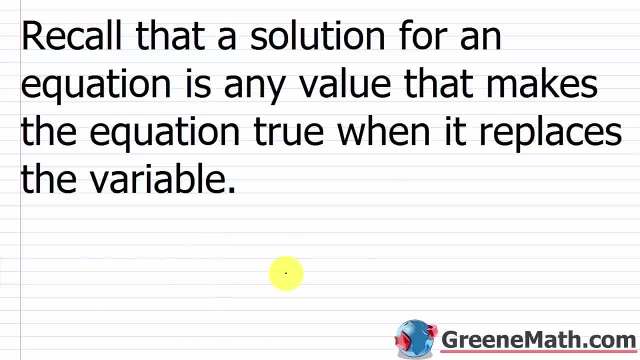 Just remember that and it'll make it easy for you to write it out each time. Now let's kinda move into the main part of the lesson. We're gonna start solving these quadratic equations using factoring, So I want you to first recall that a solution. 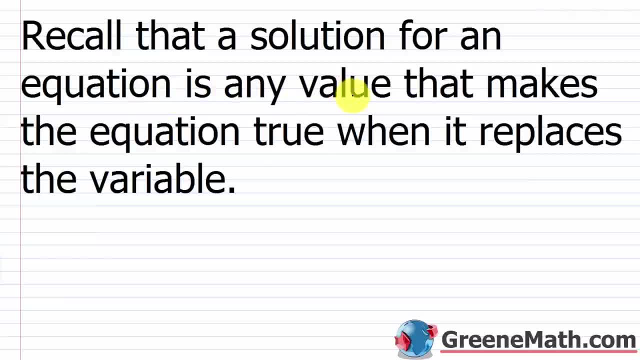 for an equation is any value, or it could be values. that makes the equation true when it replaces the variable, or it could be variables if you have more than one. So, for example, if we think back to when we're working with linear equations, we have three x minus five. 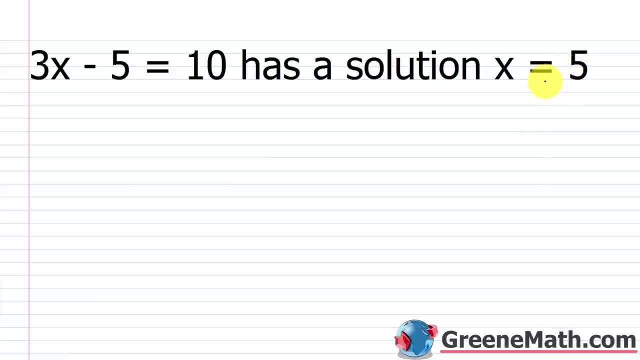 equals 10, I have here that this has a solution of x equals five. Why? Because if I plug a five in for x, there I get a true statement. If I take three and I multiply it by five minus five equals 10, three times five is 15,. 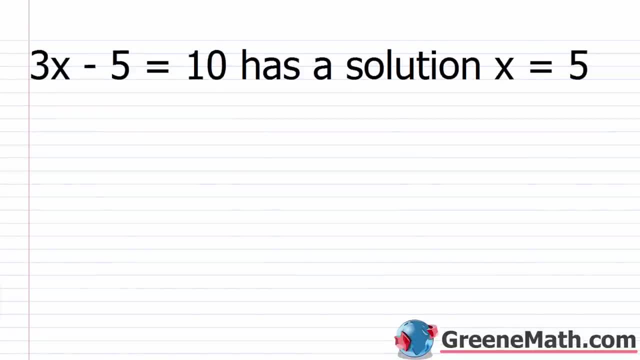 So for example, if we think back to when we're working with linear equations, we have three x minus five equals 10. 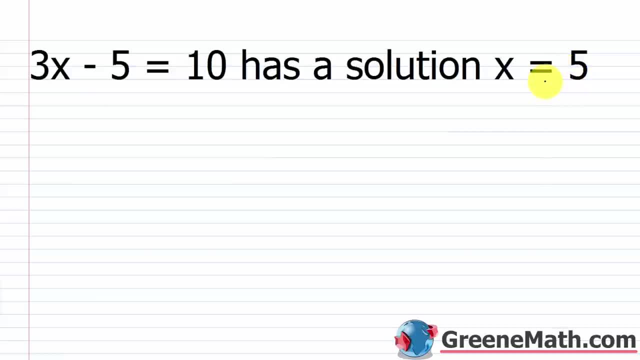 I have here that this has a solution of x equals five. Why? 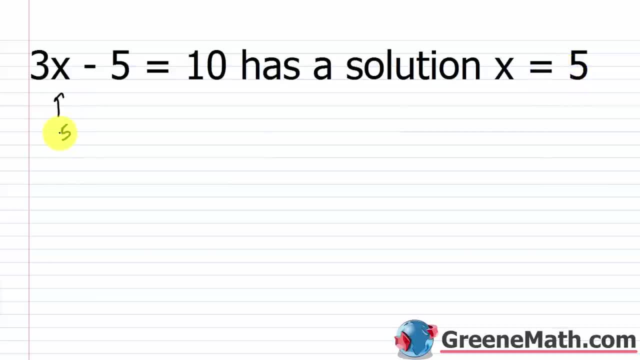 Because if I plug a five in for x there, I get a true statement. If I take three and I multiply it by five, minus five equals 10. Three times five is 15, I get 15 minus five equals 10. And then I get 10 equals 10. So the left and the right side are the same value. And so this equation is now true, right? 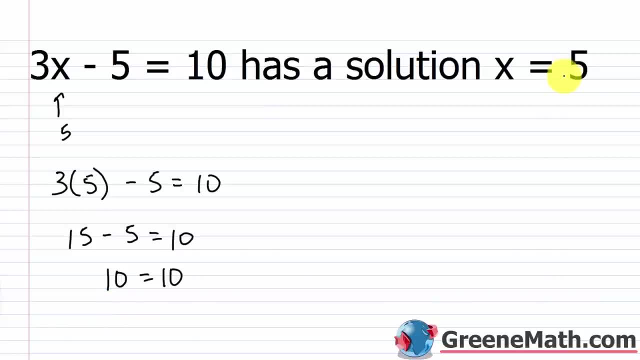 But it's only true if x is equal to five, it's not true for any other value of x. And then let's look at one other one. 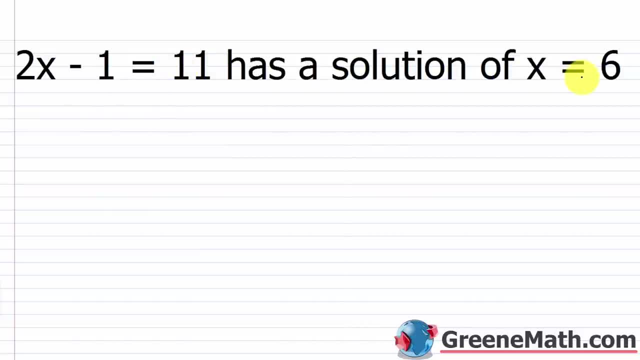 We have that two x minus one equals 11 has a solution of x equals six. Again, if I put a six in for x, I would have two times six minus one equals 11. We could see that would work out two times six is 12 minus one equals 11. We get 11 equals 11. Again, same value on the left and the right side. So we know that x equals six is the correct solution. 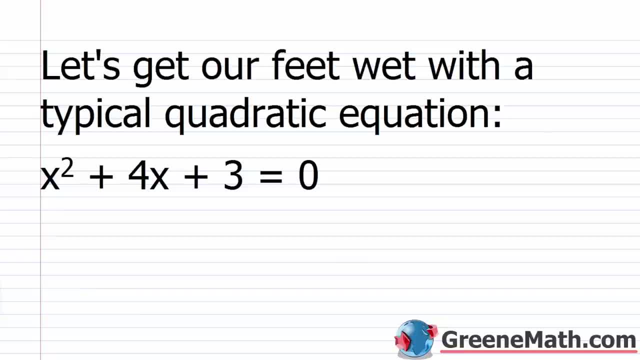 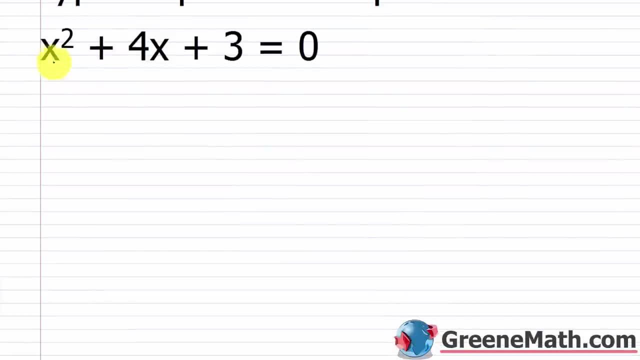 All right, so let's get our feet wet with a typical quadratic equation. So you'll notice that it's set up for us in what we call, again, standard form. So we have x squared plus four x plus three. 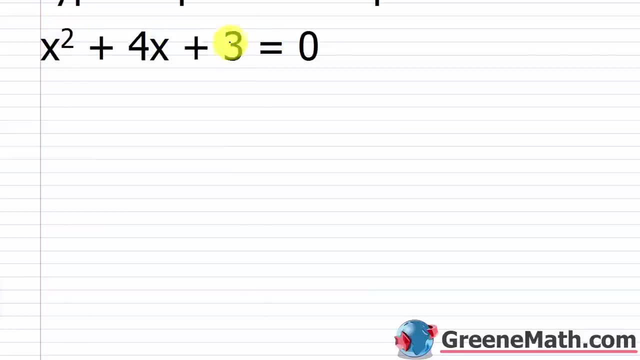 So it's an exponent of two, it's an exponent of one, and you kind of think about your constant term there. So it goes in descending order of powers. 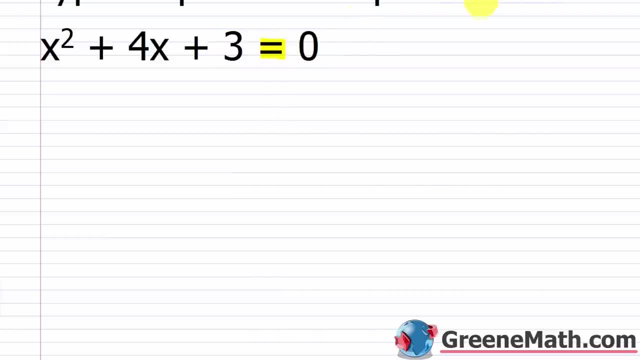 And then again, notice how we've set it equal to zero. So if something's equal to zero, you're going to see that we can use a special property for this. 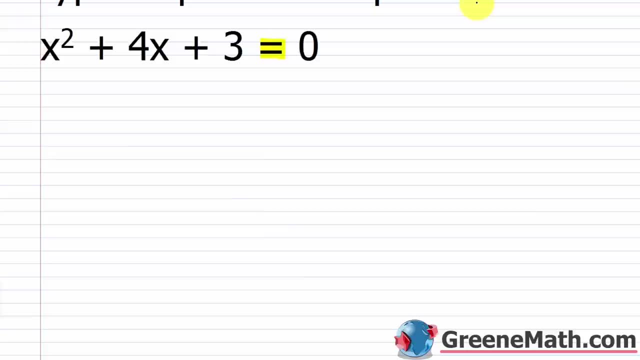 So the first thing I want you to do is I want you to factor this guy. So we know how to factor a triangle. We know how to factor a binomial. 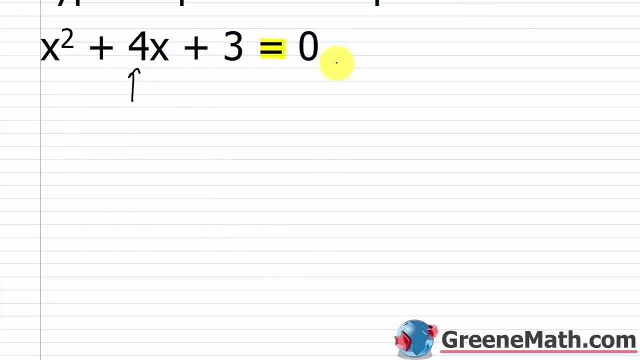 And that's what the left side of this is. Left side of the trinomial, right side is zero. 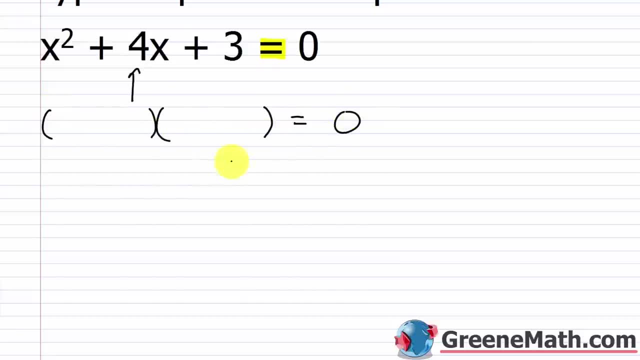 So I'm going to set this up into two binomials. And so I know I'm going to have x here and x here. And these are both positive, so plus something and plus something else. 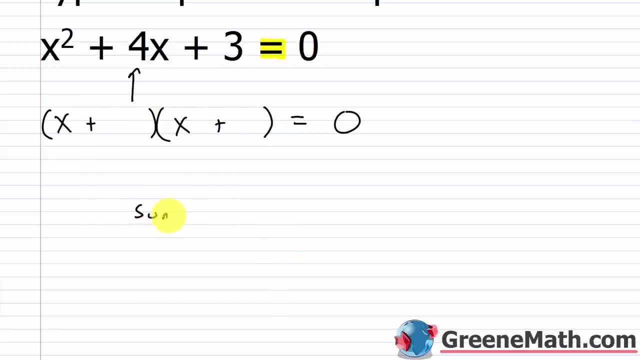 And just give me two integers whose sum is what? Is four, right? 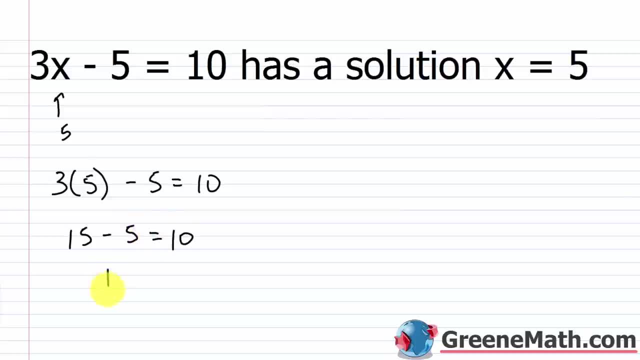 I'd get 15 minus five equals 10.. And then I get 10 equals 10.. So the left and the right side are the same value, and so this equation is now true. Right, but it's only true if x is equal to five. 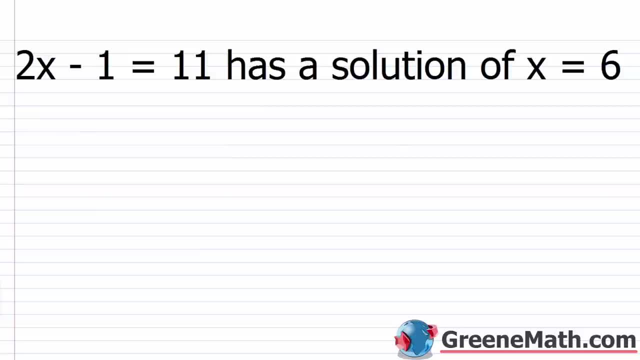 It's not true for any other value of x. And then let's look at one other one. We have that two x minus one equals 11 has a solution of x equals six. Again, if I put a six in for x, I would have two times six minus one equals 11.. 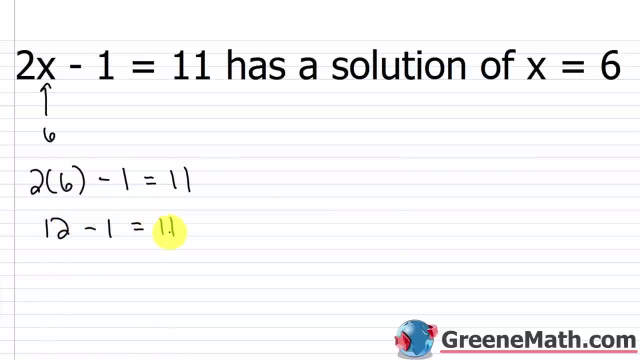 We could see that would work out: two times six is 12, minus one equals 11.. We'd get 11 equals 11. Again, same value on the left and the right side. So we know that x equals six is the correct solution. 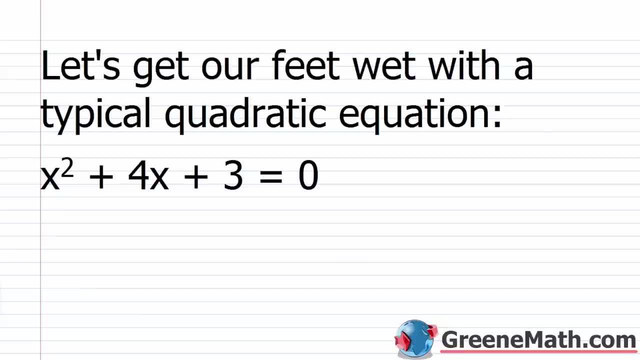 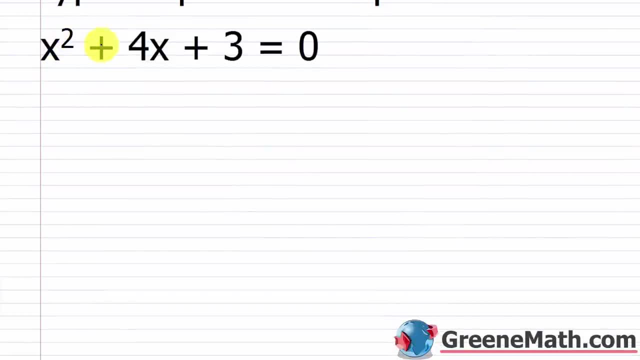 All right, so let's get our feet wet with a typical quadratic equation. So you'll notice that it's set up for us in what we call again standard form. So we have x squared plus four, x plus three, So it's an exponent of two, it's an exponent of one. 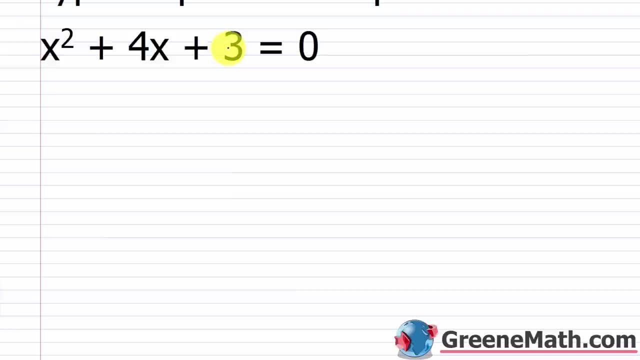 and you kind of think about your constant term there. So it goes in descending order of powers. And then again notice that it's a constant term, So it goes in descending order of powers. Notice how we've set it equal to zero. 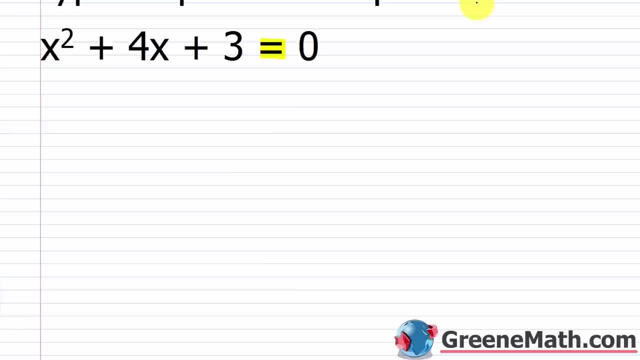 So if something's equal to zero, you're gonna see that we can use a special property for this. So the first thing I want you to do is I want you to factor this guy, So we know how to factor a trinomial. 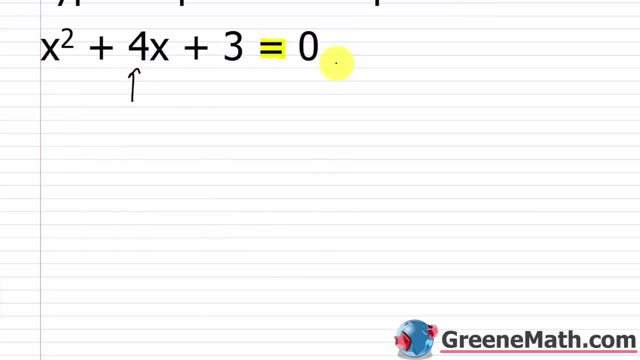 and that's what the left side of this is. Left side's a trinomial, right side is zero. So I'm gonna set this up into two binomials, And so I know I'm gonna have x here and x here. 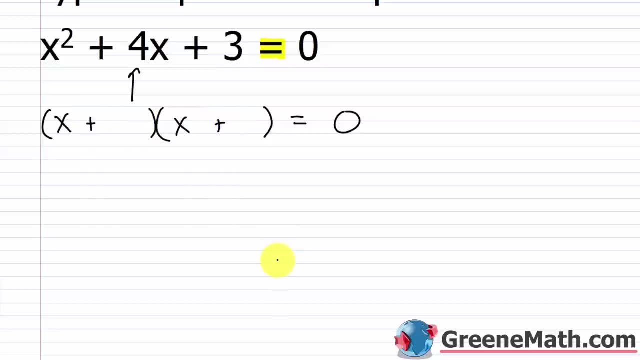 And these are both positives. so plus something and plus something else. And just give me two integers whose sum is what Is four right? The coefficient for the x to the first power. We generally refer to this as b right. Remember we say ax squared plus bx plus c. 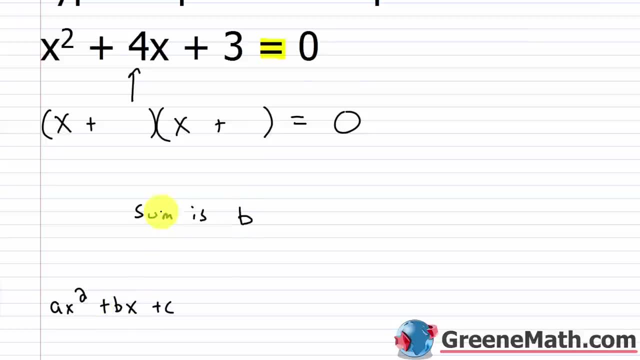 The coefficient for the x to the first power. we generally refer to that as b, So the sum is b and the product the product is c. right, That constant term, which in this case is three. So b here is four. 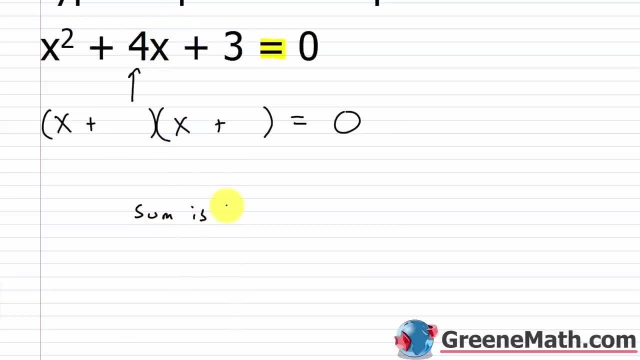 The coefficient for the x to the first power. We generally refer to this as b, right? Remember, we say ax squared. 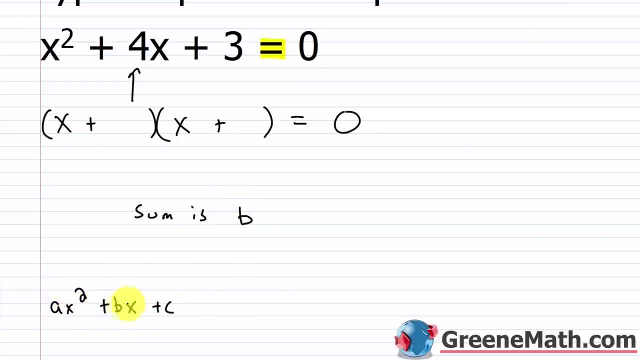 Plus bx plus c. The coefficient for the x to the first power, we generally refer to that as b. So the sum is b and the product, the product is c, right? That constant term, which in this case is three. So b here is four, c here is three. So give me two numbers whose sum is four and whose product is three. Well one and three, right? If you think about the factors of three, three is a prime number. So without going into any negatives. 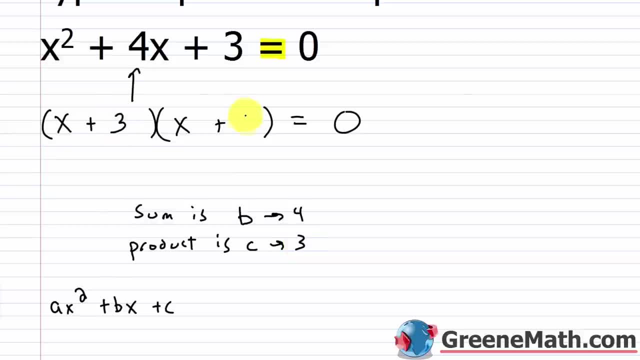 You just have three times one. So three and one. And three plus one does give you four. 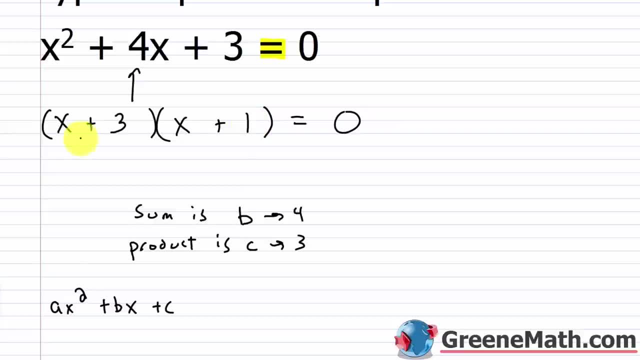 So that would work out. And you can check it through FOIL if you want. X times x is x squared. The outer would be x. The inner would be three x. X plus three x is four x. That would give you the middle. 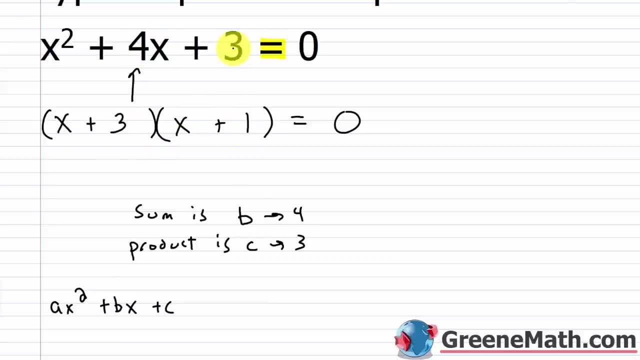 And then three times one is three. That would give you your last term there. So we factored this correctly. 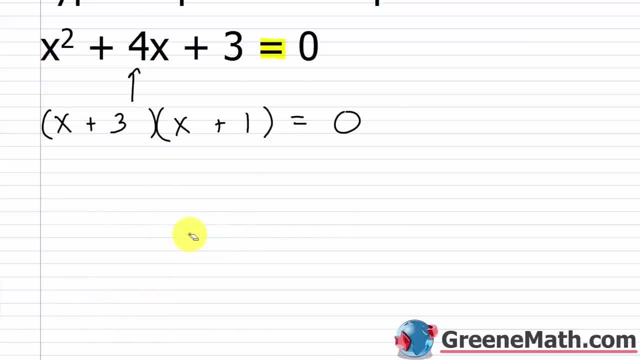 Now once we've factored this correctly, what do we do? We have a binomial times another binomial. We have a binomial times another binomial equal to zero. So in order to solve this type of problem, I'm going to introduce something known as the zero product property. 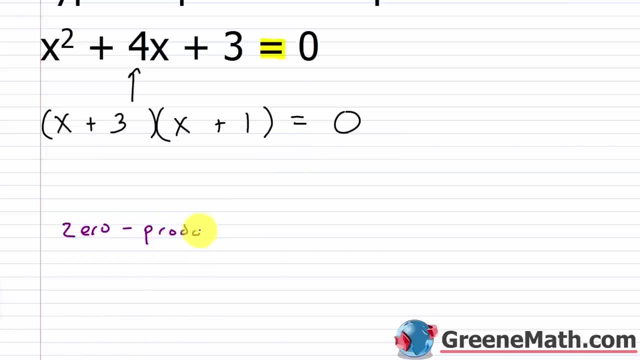 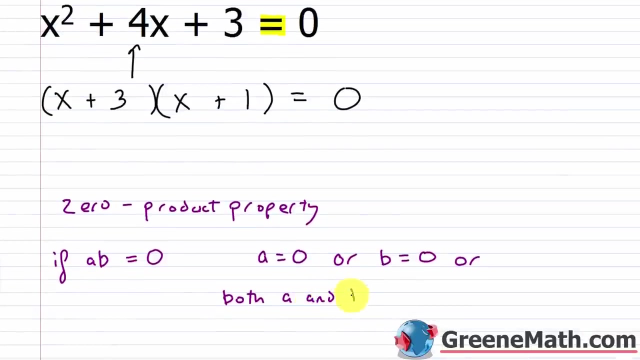 So the zero product property. And this tells us that if a times b is equal to zero. And when I say a times b, I mean any real number a times any real number b. So two numbers being multiplied together. So if a times b is equal to zero, then what could be the possible answers for a and for b? Well, a could be equal to zero, or b could be equal to zero, or both a and b are equal to zero. Those three scenarios. 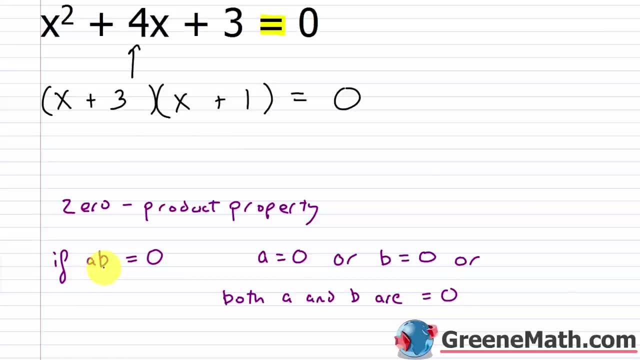 Because when I multiply a number times zero, I get zero as a result. So a could be any number. That's not zero. 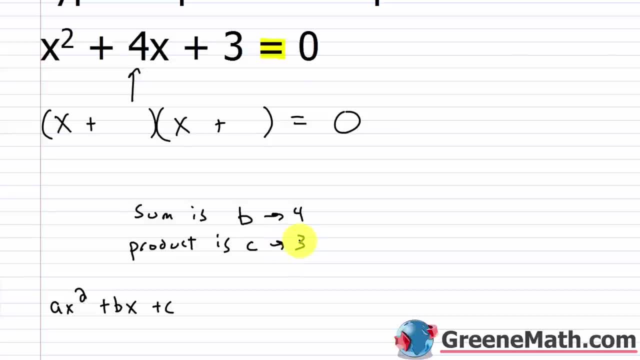 C, here is three. So give me two numbers whose sum is four and whose product is three. Well, one and three, right? If you think about the factors of three, three's a prime number. So, without going into any negatives, you just have three times one. 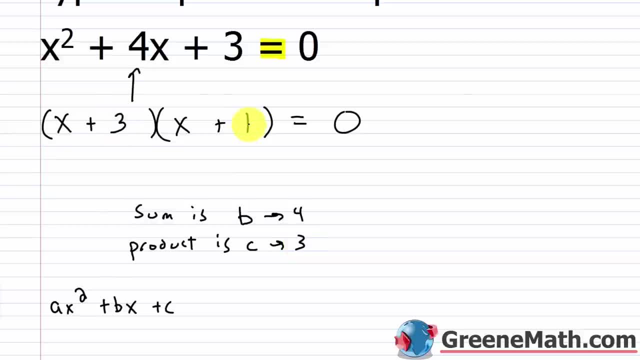 So three and one and three plus one does give you four. So that would work out And you can check it through FOIL, if you want. X times x is x squared. The outer would be x, The inner would be three x. 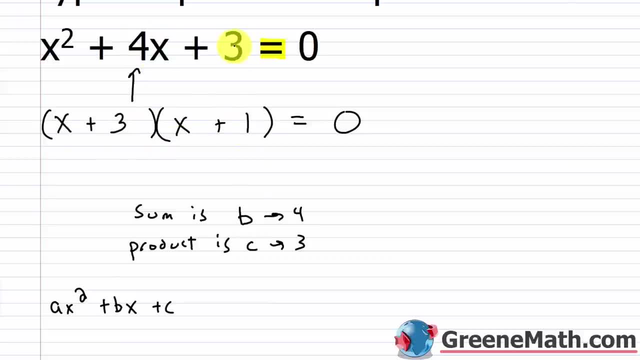 X plus three, x is four. x. That would give you the middle. And then three times one is three. That would give you your last term there. So we factored this correctly. Now, once we've factored this correctly, what do we do? 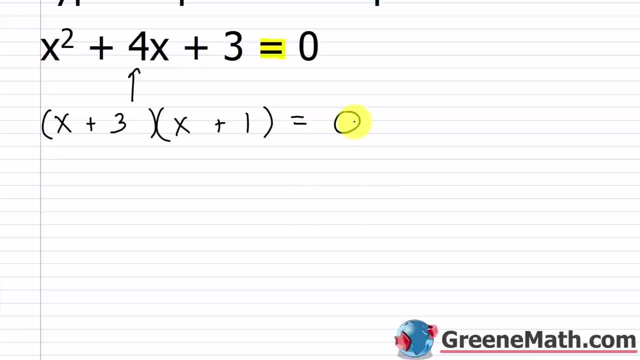 We have a binomial times another binomial equal to zero. So, in order to solve this type of problem, I'm gonna introduce something known as the zero product property, So the zero product property, And this tells us that if a times b is equal to zero, 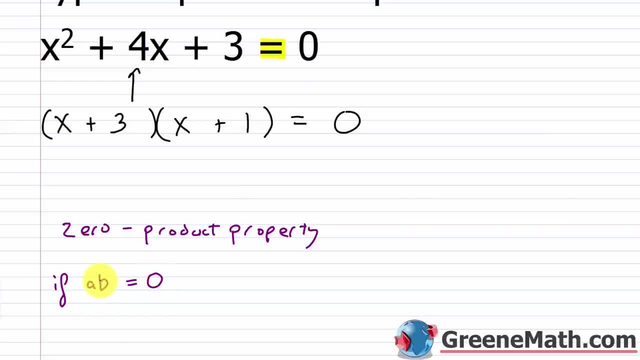 and when I say a times b, I mean any real number a times any real number, b, So two numbers being multiplied together. If that result is zero, then what could be the possible answers for a and for b? Well, a could be equal to zero. 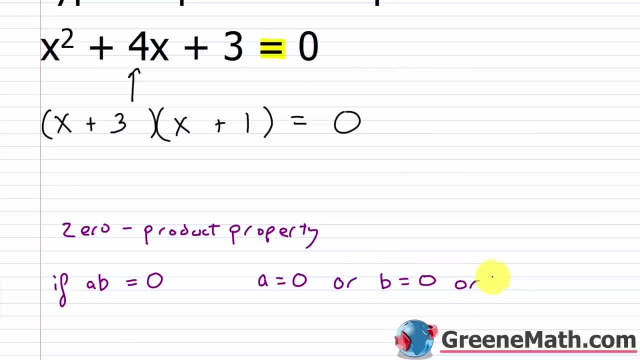 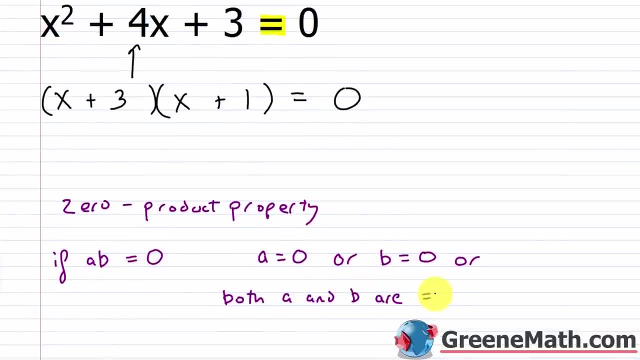 or b could be equal to zero, or both a and b Or b could be equal to zero. Those three scenarios, Because when I multiply a number times zero, I get zero as a result. So a could be any number that's not zero. 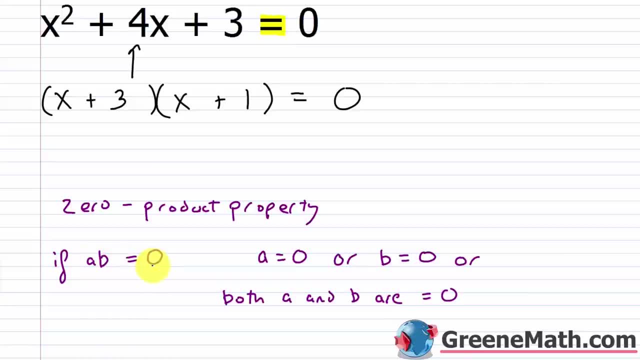 and b could be zero. When I multiply them together, I get zero. B could be any number that's not zero. A could be zero. Multiply them together: you get zero. A and b could each be zero. If I multiply zero times zero, I still get zero. 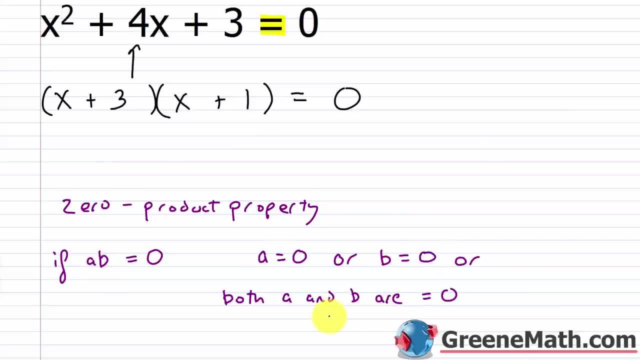 So that's where these three scenarios come from. So we've got a binomial. We can use this property to get a solution for this equation here, If I first start by realizing that x plus 3, that quantity is being multiplied by the quantity x plus 1.. 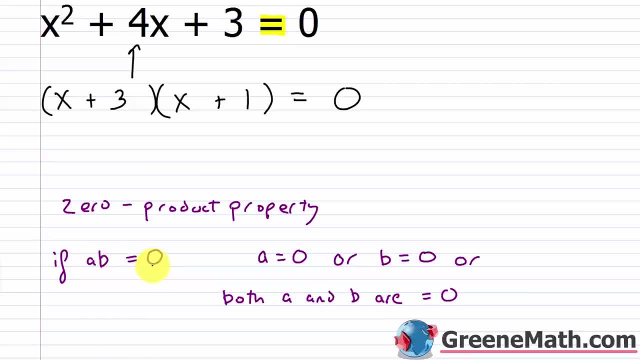 And b could be zero. When I multiply them together, I get zero. B could be any number. That's not zero. A could be zero. Multiply them together. You get zero. A and b could each be zero. 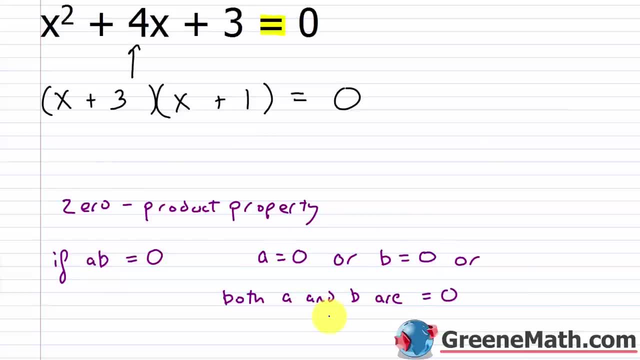 If I multiply zero times zero, I still get zero. So that's where these three scenarios kind of come from. 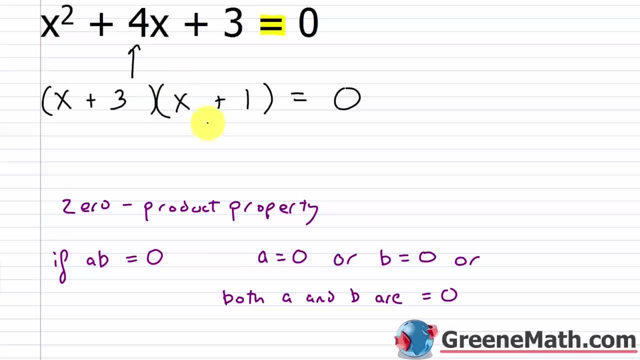 So we can use this property to get a solution for this equation here. If I first start by realizing that x plus three, that quantity is being multiplied by the quantity x plus one. Well. I've plugged in something for x there. 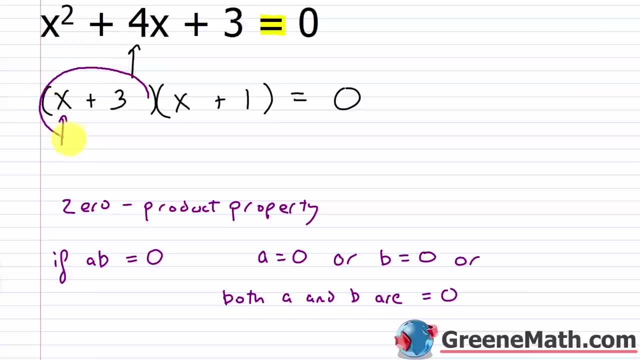 Some value. And it made this factor here, this binomial x plus three equal to zero. Then when zero is multiplied by this guy right here, it's going to give me zero. So I've found a solution for the equation. I've replaced the variable with a value that makes the equation true. So the way we utilize this is we just set each of these equal to zero separately. We'll get two solutions. And then we will check. Each solution in the original equation. 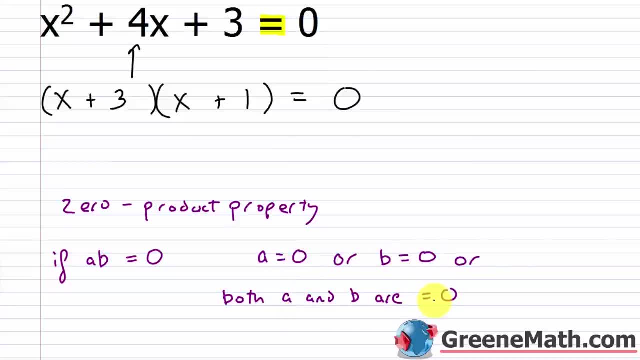 Remember. A could be zero. B could be zero. Or they both could be zero. 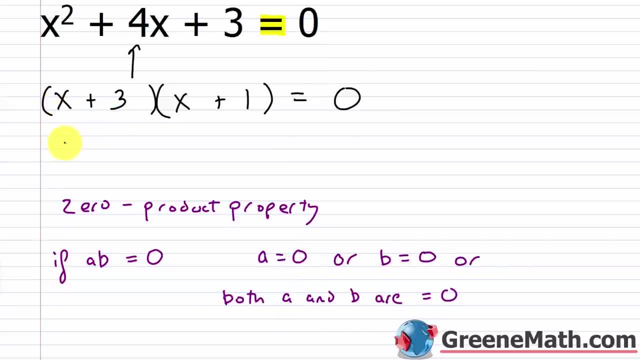 So let's start this out by just saying, okay, x plus three, x plus three is equal to zero. Very, very easy to solve that. I just subtract three away from each side of the equation. And I would get that x is equal to negative three. So this is one proposed solution. And then the other one. The other factor here. 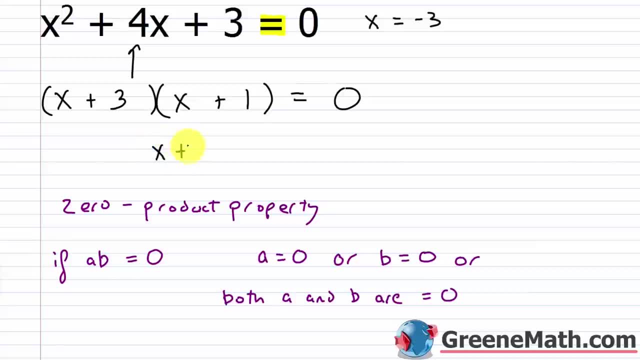 Is x plus one. So x plus one. We set that equal to zero. We'd subtract one away from each side. 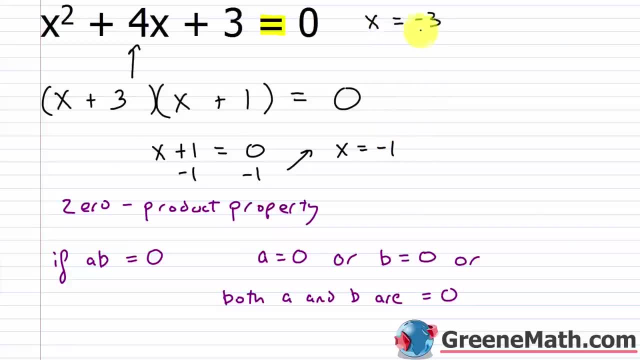 And we get that x is equal to negative one. So we put x equals negative three or x equals negative one. Could be any of those at this point. 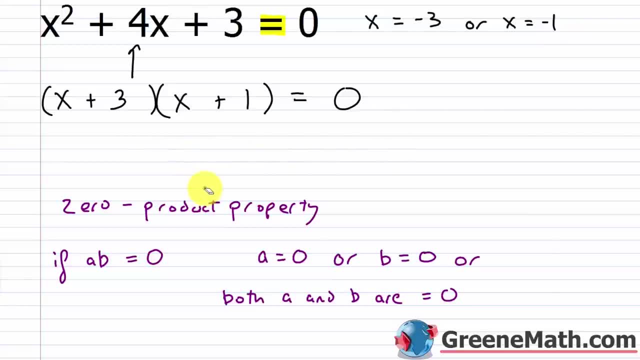 So let's erase this real quick. And I can show you why this works. 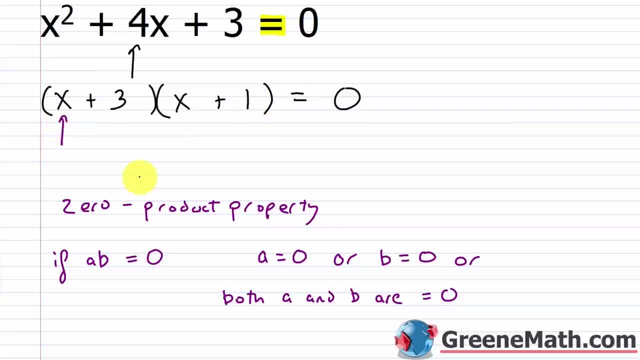 Well, if I plugged in something for x there some value, and it made this factor here, this binomial x plus 3, equal to zero, then when zero is multiplied by this guy right here, it's going to give me zero. 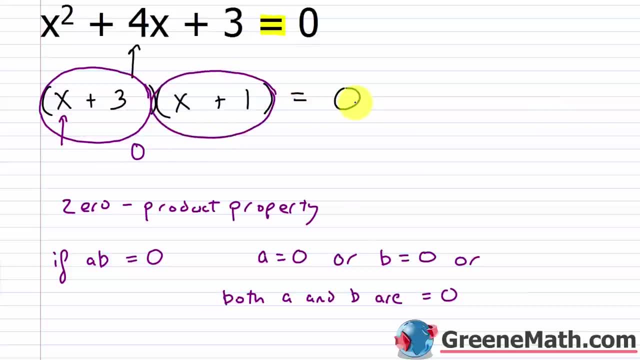 So I've found a solution for the equation. I've replaced the variable with a value that makes the equation true. So the way we utilize this is we just set each of these equal to zero separately. We'll get two solutions and then we will check each solution. 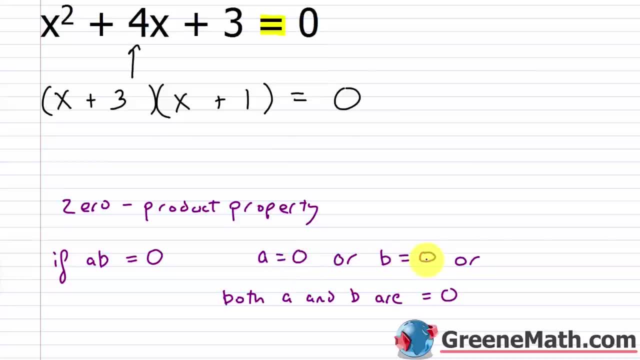 in the original equation, Remember, a could be zero, b could be zero or they both could be zero. So let's start this out by just saying: OK, x plus 3,. x plus 3, is equal to zero. 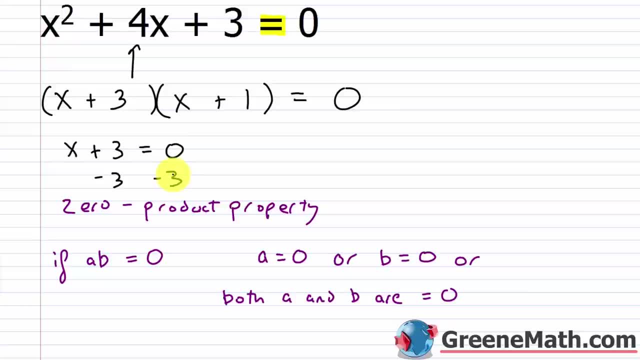 Very, very easy to solve that. I just subtract three away from each side of the equation And I would get that x is equal to negative 3.. So this is one proposed solution And then the other one. the other factor here is x plus 1.. 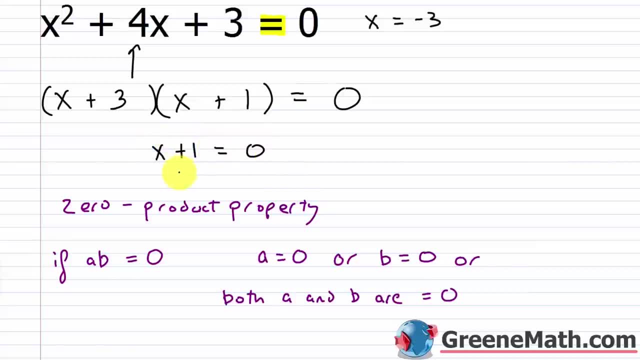 So x plus 1, we set that equal to zero. We'd subtract one away from each side and we get that x is equal to negative 1.. So we put x equals negative 3, or x equals negative 1.. Could be any of those at this point, 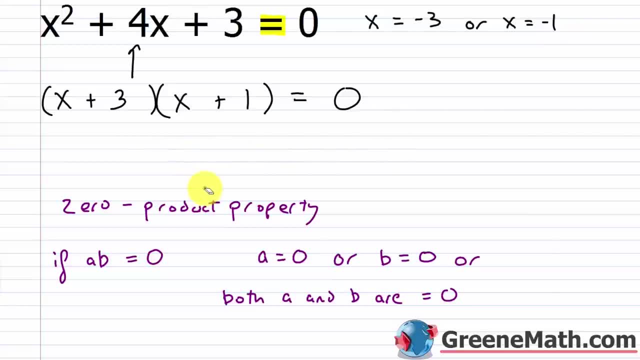 So let's erase this right here. OK, Let's erase this real quick And I can show you why this works. So let me erase all this. So, without going back into the very original x squared plus 4x plus 3 equals 0, which we'll. 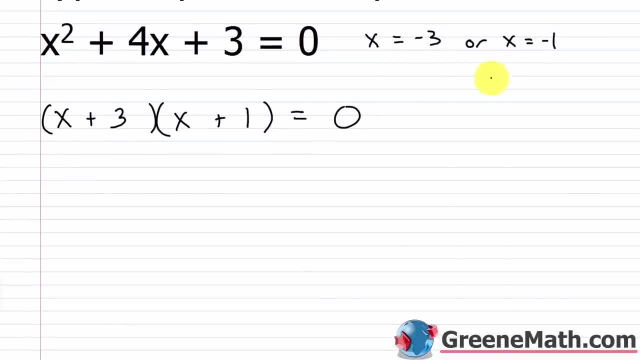 do in a minute. I want to show you in this format here how this plays out. I think it'll give you a better understanding. So we have the quantity x plus 3, that is being multiplied by the quantity x plus 1. This is supposed to be equal to zero. 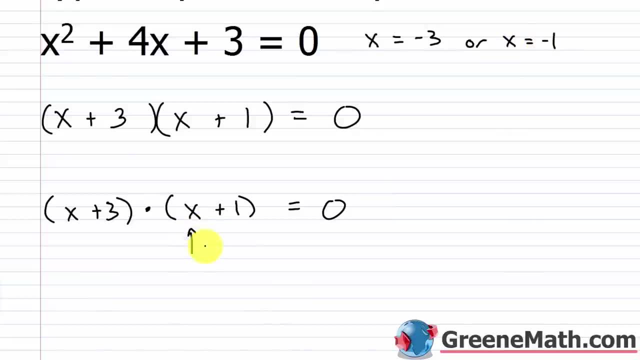 So let's start out by just plugging in a negative 1 for x here. So if I plugged in a negative 1 there and a negative 1 there, what would happen? Well, negative 1 plus 1 is zero. We found that out by setting x plus 1 equal to zero and solving for x. 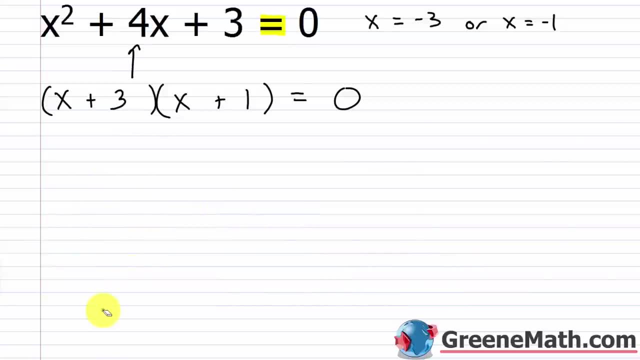 So let me, let me erase all this. So without going back into the very original x squared plus four x plus three equals zero, 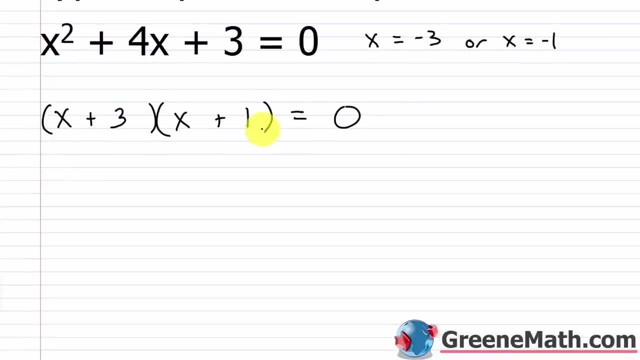 which we'll do in a minute, I want to show you in this format here, how this plays out. I think it'll give you a better understanding. 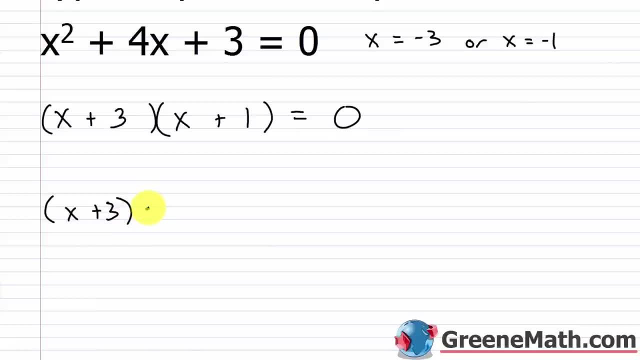 So we have the quantity x plus three that is being multiplied by the quantity x plus one. This is supposed to be equal to zero. 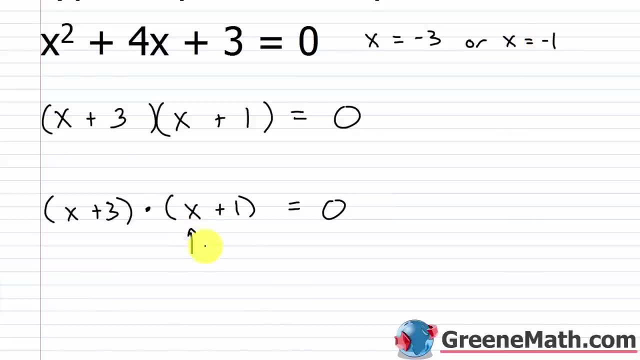 So let's start out by just plugging in a negative one for x here. So if I plugged in a negative one there and a negative one there, what would happen? Well, negative one plus one is zero. We found that out. So we're going to start by putting x plus one equal to zero and solving for x. 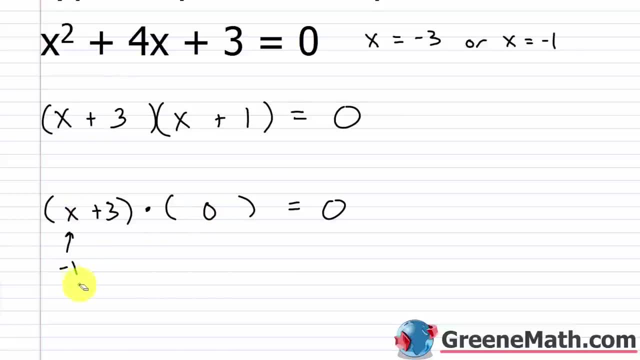 So this would be zero. And then if I plugged in a negative one here, negative one plus three is two. Well there you go. Zero times two is zero. So that's how that works, right? 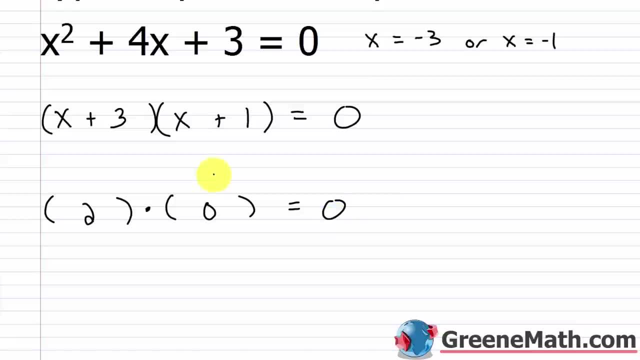 Anything times zero gives you zero. So all I need is one of these factors to be zero and I'll get a true statement. 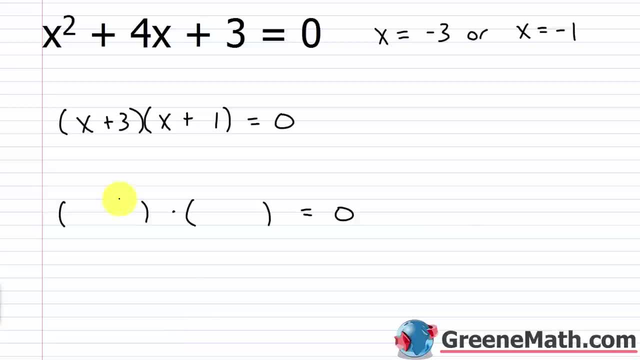 So now let me show you what happens with x equals negative three. So again, let me just write x plus three, that quantity here, and it's multiplied by, again, let me write x plus one, that quantity there, and I'm going to plug in a negative three now. So I'm going to plug in a negative three here and then also here. And you're going to see the same thing happen. 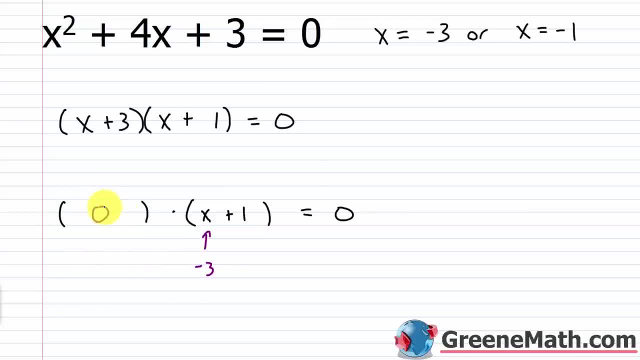 Negative three plus three is zero. So I have one factor that's zero. And then negative three plus one is negative two. So this is negative two. And zero times anything is zero. So zero times negative two is, of course, zero. So again, we'll get a true statement. 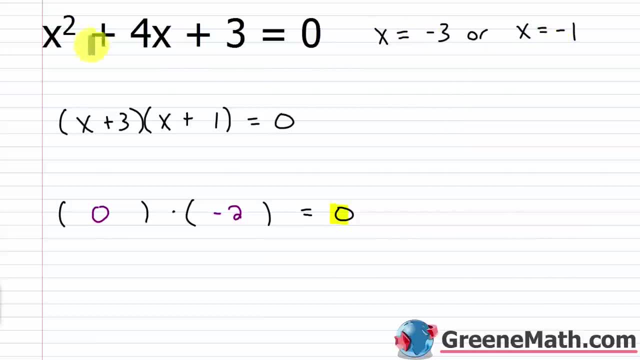 And I'm going to show you that these two solutions work in the original equation that's not factored. 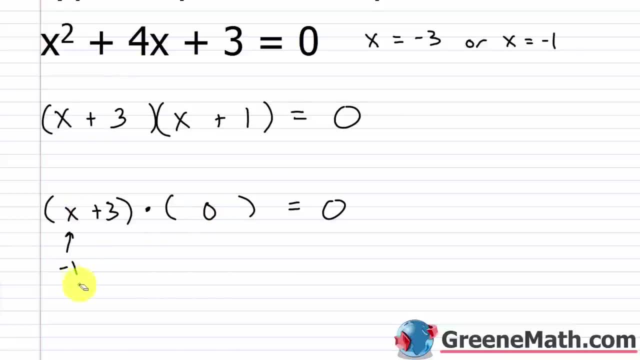 So this would be zero. And then, if I plugged in a negative 1 here, negative 1 plus 3 is 2.. Well, there you go. Zero times 2 is zero. So that's how that works, right? Anything times zero gives you zero. 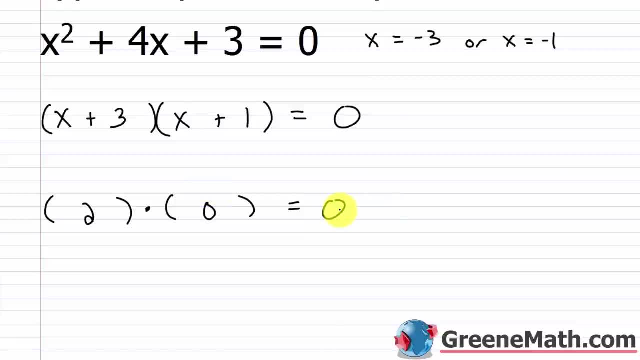 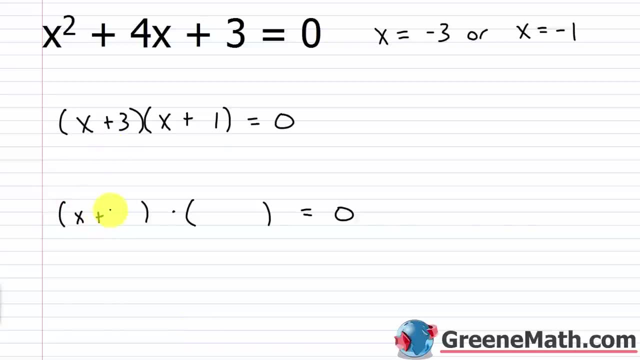 So all I need is one of these. I want all of these factors to be zero and I'll get a true statement. So now let me show you what happens with. x equals negative 3.. So again, let me just write x plus 3, that quantity here, and this is multiplied by. 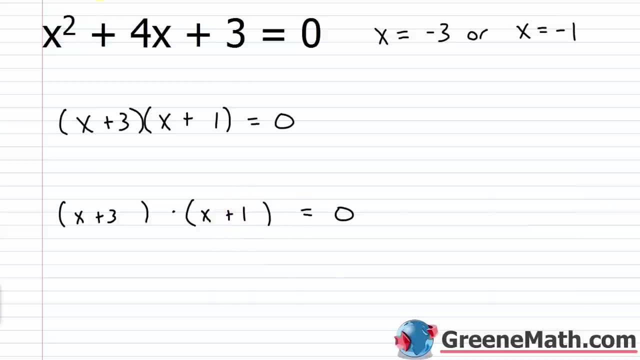 again, let me write x plus 1, that quantity there, and I'm going to plug in a negative 3 now. So I'm going to plug in a negative 3 here and then also here, And you're going to see the same thing happen. 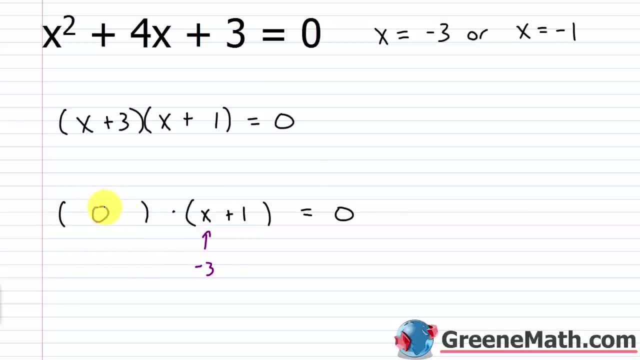 Negative 3 plus 3 is zero. So I have one factor that's zero, And then negative 3 plus 1 is negative 2.. So this is negative 2.. And zero times anything is zero. So zero times negative 2 is of course zero. 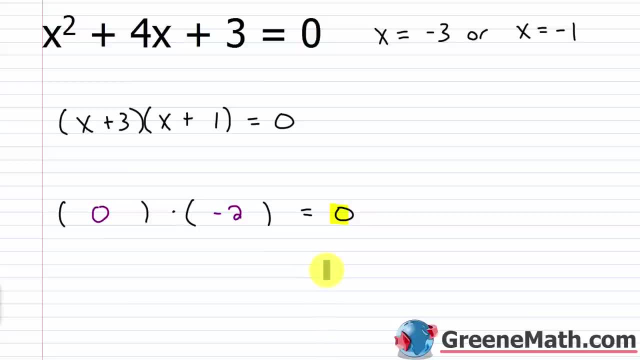 So again we'll get a true statement. So let's erase everything here And I'm going to show you that these two solutions work. in the original equation that's not factored. So if I plugged in a negative 3 here and here we're starting with this one, 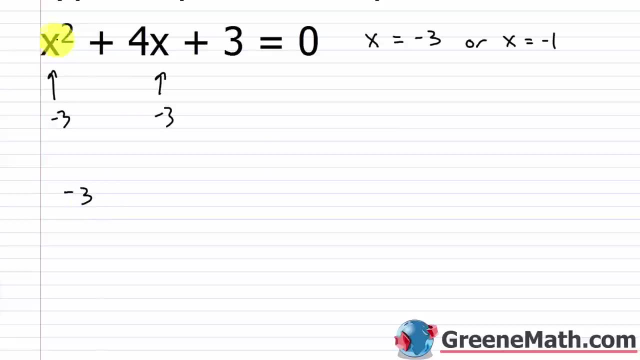 So we would have negative 3, that quantity You're plugging in for x and x is squared, So you've got to use parentheses there So that quantity is squared plus 4 times negative 3, plus 3, and this should be equal. 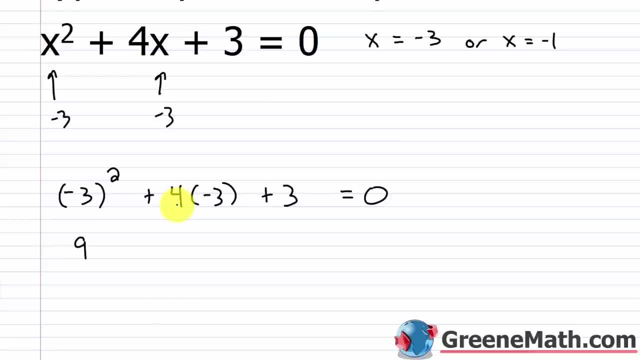 to zero. Negative. 3 squared is 9, 4 times negative. 3 is negative 12,. so minus 12, plus 3 equals zero. 9 plus 3 is 12,. 12 minus 12 is zero. So this is zero equals zero. 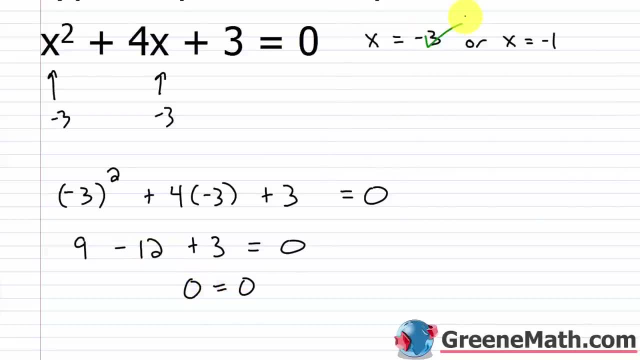 So that checks out as a solution. And then x equals negative 1.. Let's do the same thing with negative 1.. Erase this, So we'd have negative 1 squared, that's 1.. And then 4 times negative 1 is negative 4, so minus 4, and then plus 3, and this equals. 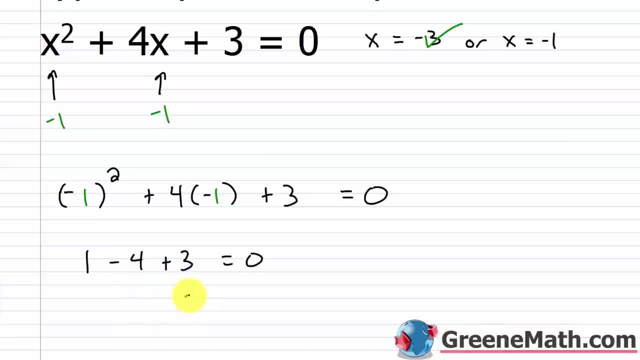 zero 1 minus 4 is negative 3, negative 3 plus 3 is zero. so you get zero equals zero, So that one checks out as well, And so my solution is: x equals negative 3, or it could also be that x equals negative. 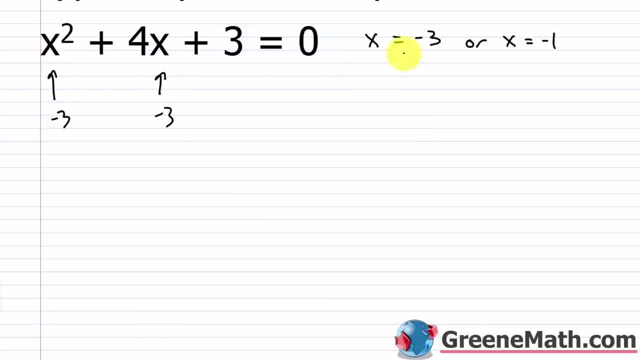 So if I plugged in a negative three here and here, we're starting with this one. So we would have negative three, that quantity. You're plugging in for x and x is squared, so you got to use parentheses there. So that quantity is squared plus four times negative three plus three, and this should be equal to zero. 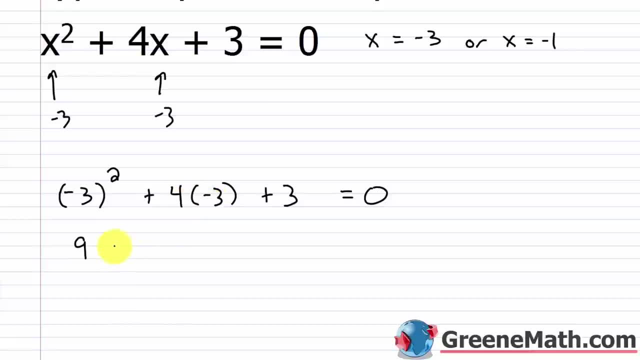 Negative three squared is nine. Four times negative three is negative 12. So minus 12 plus three equals zero. Nine plus three is 12. 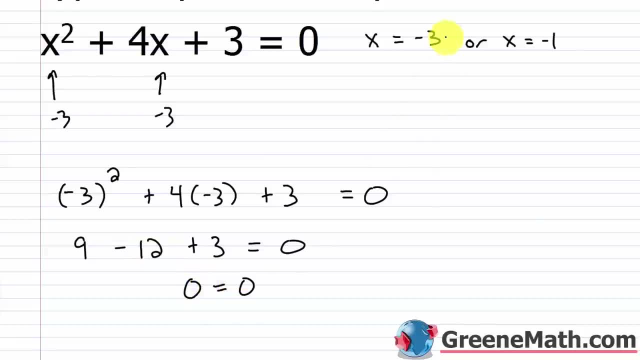 12 minus 12 is zero. So this is zero equals zero. So that checks out as a solution. 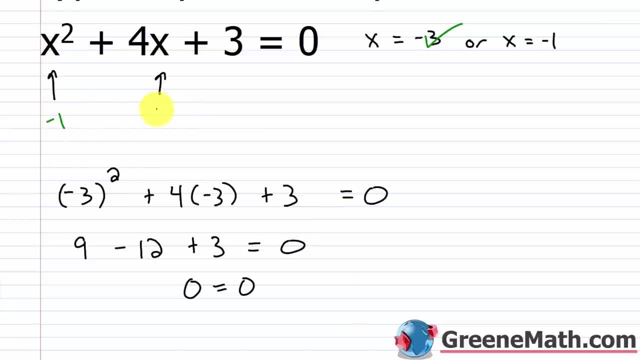 And then x equals negative one. Let's do the same thing with negative one. Erase this. 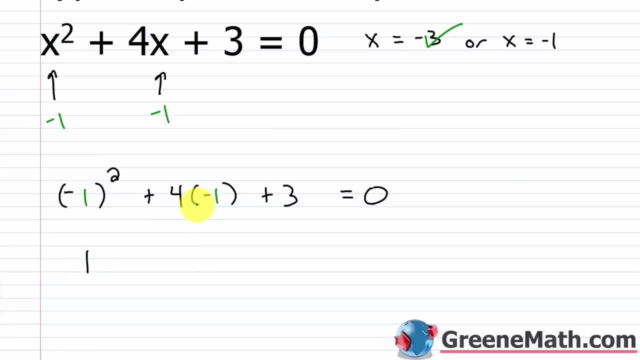 So we'd have negative one squared. That's one. And then four times negative one is negative four. So minus four. And then plus three. 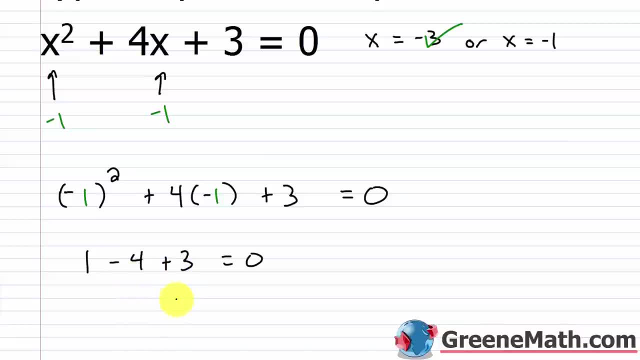 And this equals zero. One minus four is negative three. Negative three plus three is zero. So you get zero equals zero. So that one checks out as well. 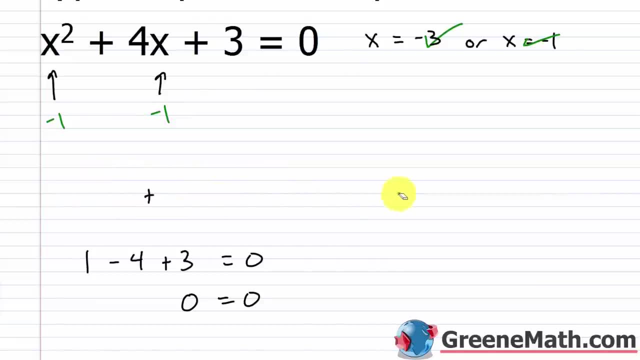 And so my solution is x equals negative three, or it could also be that x equals negative one. 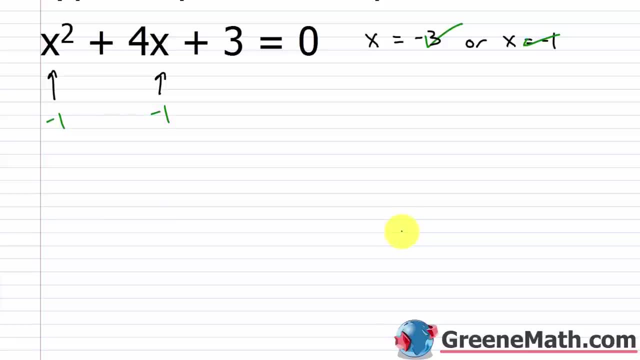 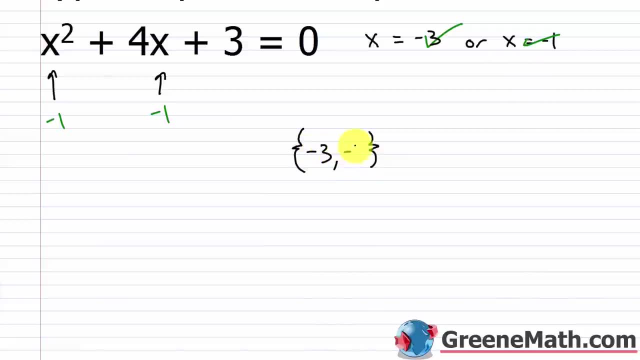 So in this case, you'd have negative three comma negative one. But in algebra one this is still pretty much acceptable. So either way you want to write your solution, either with the solution set notation which will cover greatly in Algebra Two, or with this notation here that we've been using forever, as long as you're displaying to you teacher what the solution is. You Damen us zero here. 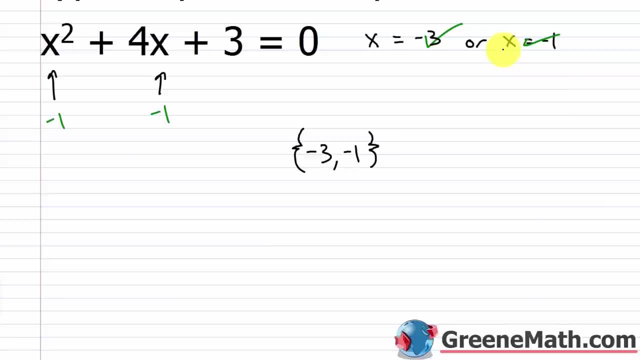 negative 3 or x can be negative 1 and those solutions are correct you should get full credit 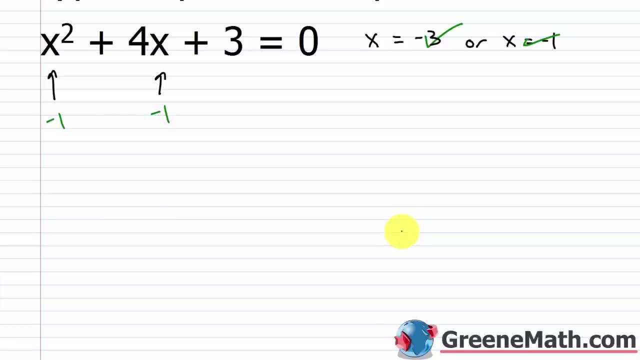 1. Either way those would work, And typically in an Algebra 1, or later on in Algebra 2, you're going to write this using something known as a solution set, So it's set braces which look like this: 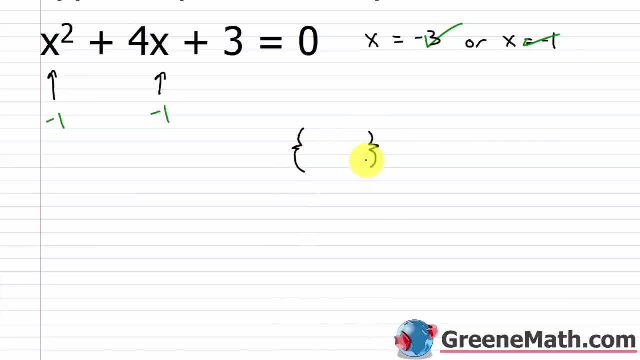 And inside of the set braces you would list your solutions for that equation. So in this case you'd have negative 3, comma, negative 1.. But in Algebra 1, this is still pretty much acceptable. So either way you want to write your solution. 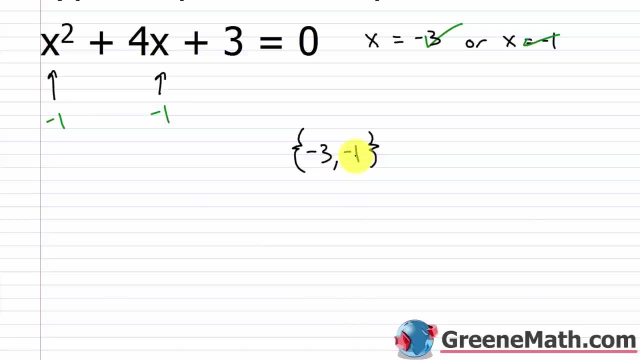 Either with the solution set notation, which will cover greatly in Algebra 2, or with this notation here that we've been using forever, as long as you're displaying to your teacher what the solution is: x could be negative 3, or x could be negative 1, and those solutions 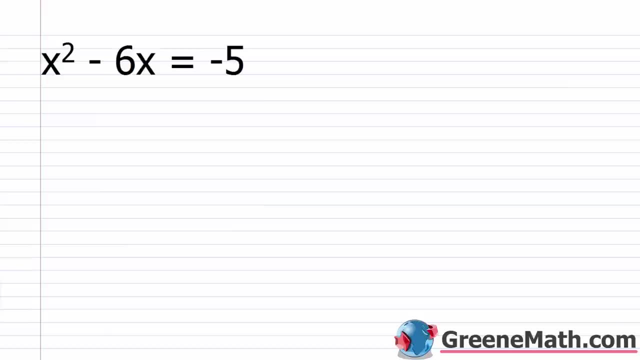 are correct, you should get full credit, All right. so let's take a look at another one, And I want to just cover the full procedure with you on this one, And the very first thing you always want to do if you're going to solve a quadratic equation. 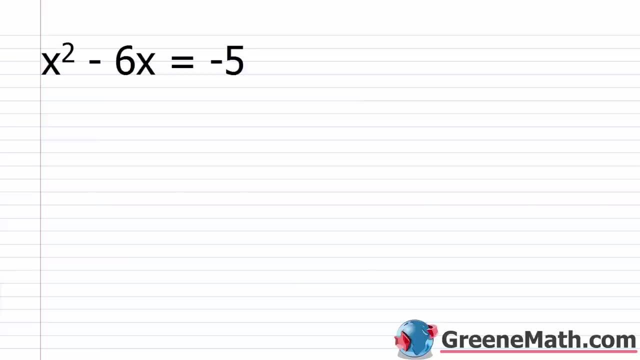 by factoring. You want to start out by pulling, By putting the left side of the equation as ax squared plus bx plus c. The right side of the equation should be 0.. So, in other words, with this, x squared minus 6x equals negative 5, I would add 5 to both. 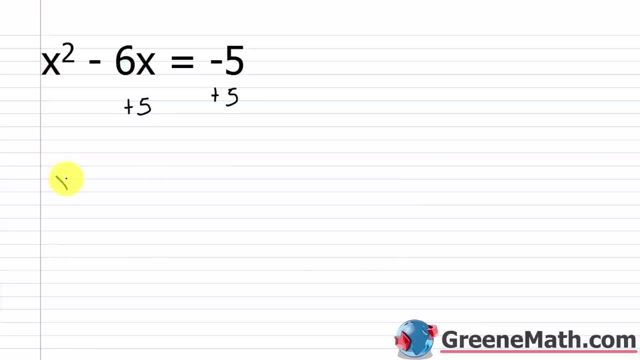 sides of the equation. And what's that going to give me? It's going to give me x squared minus 6x plus 5.. And this is equal to, if I have negative 5 plus 5, that gives me 0.. 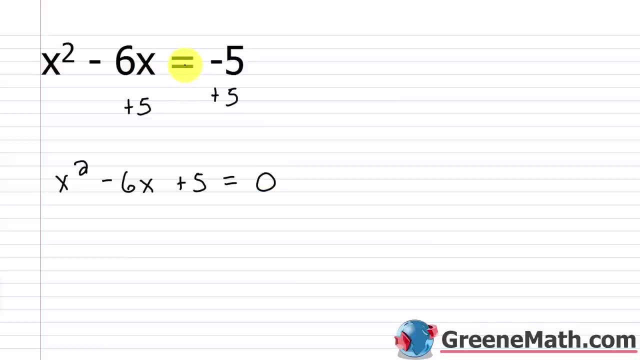 So I've got to write 0.. The only mistake is they forget to have this equal sign here and they just don't write anything after they do that. So they're stuck and they're like: well, what do I do now? You have equal 0 there. 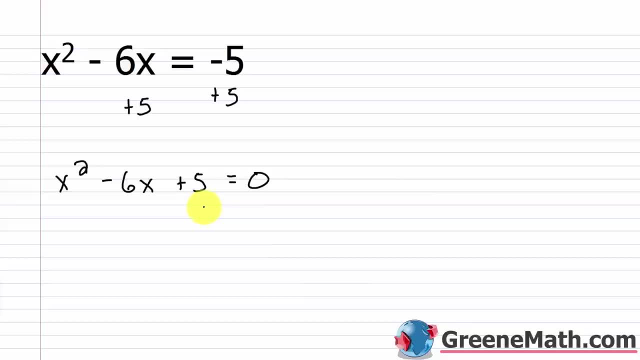 So once we've done that, we're going to factor the left side completely. In most cases that's going to be as the product of two binomials. Now, sometimes it will be slightly different if you have more factoring involved, But usually this is going to turn out to be two binomials being multiplied together and 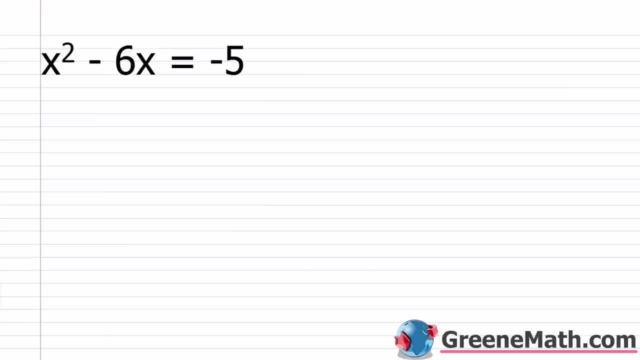 all right so let's take a look at another one and i want to just cover the full procedure with you on this one and the very first thing you always want to do if you're going to solve a quadratic equation by factoring you want to start out by putting the left side of the equation as ax squared plus bx plus c the right side of the equation should be zero so in other words with this x squared minus 6x equals negative 5 i would add 5 to both sides of the equation and what's that going to give me it's going to give me x squared minus 6x plus 5 and this is equal to if i have negative 5 plus 5 that gives me zero so i've got to write zero where students make a mistake is they forget to have this equal sign here and they just don't write anything after they do that so 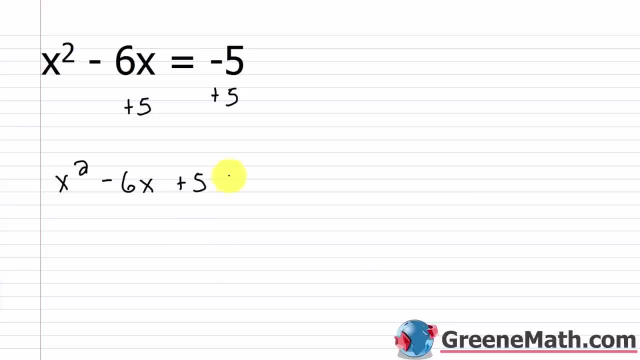 they're stuck and they're like well what do i do now you have equal zero there so once we've done that we're going to factor the left side completely in most cases that's going to be as the product of two binomials now sometimes it'll be slightly different if you have more factoring involved but usually this is going to turn out to be two binomials being multiplied together and it's set equal to zero so in this case i know it will be x here and x here we just 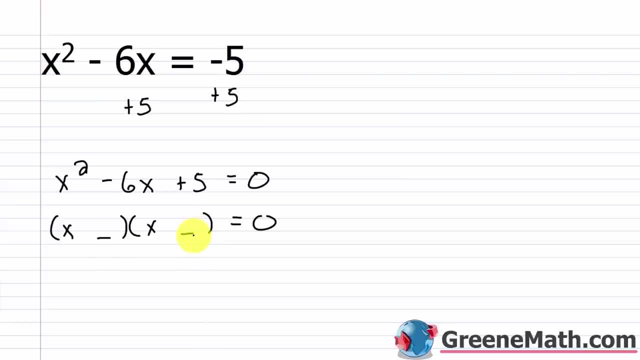 have to figure out these two missing parts here and here now once you're done with that you're going to set each factor equal to zero just like we did in the last example and then you're going to check each solution in the original equation so all i need to do here is find two integers whose sum is negative six and whose 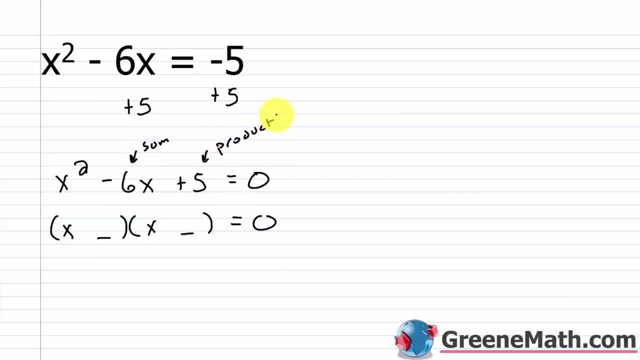 product is five so for the factors of five i know that it's a prime number so it's one times five and that's not going to work because of the sign so i got to think about negatives i could do negative one times negative five and that would sum to negative six so this would be minus one and minus five so once i've figured out what the factoring is i just set each factor remember x minus one that whole thing let me kind of do this in different parentheses that whole thing is a factor and then this guy over here let me do that in different parentheses that x minus five that 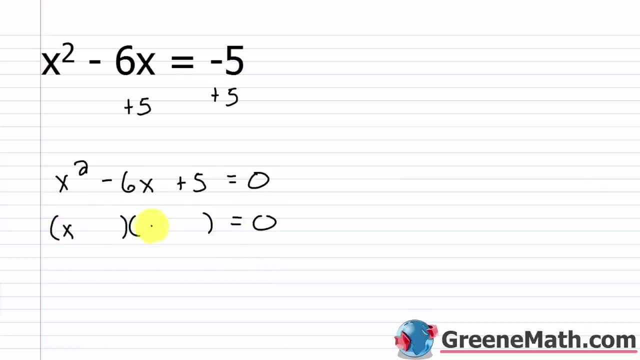 it's set equal to 0.. So in this case, I know it will be x here and x here. We just have to figure out these two missing parts here and here. Now, once you're done with that, you're going to set each factor equal to zero. 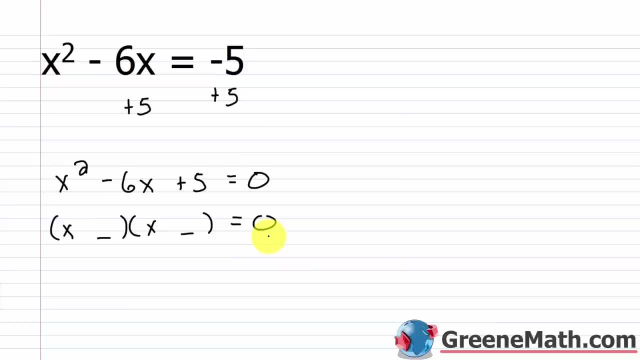 just like we did in the last example, And then you're going to check each solution in the original equation. So all I need to do here is find two integers whose sum is negative 6, and whose product is 5.. So for the factors of 5, I know that it's a prime number, so it's 1 times 5.. 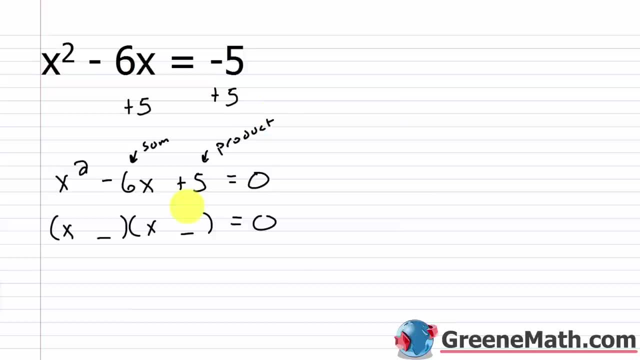 And that's not going to work because of the sign. so I've got to think about negatives. I could do negative 1 times negative 5, and that would sum to negative 6.. So this would be minus 1 and minus 5.. 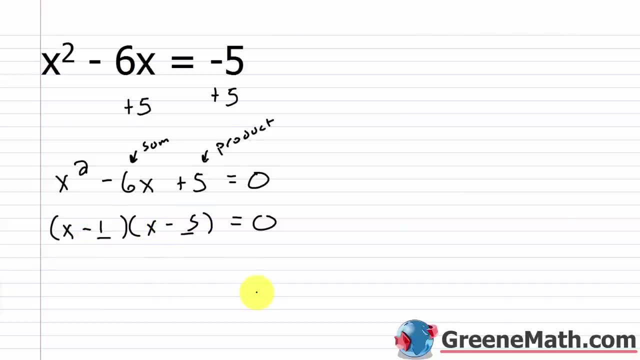 So once I've figured out what the factoring is, I just set each factor, remember x minus 1, that whole thing. let me kind of do this in different parentheses. that whole thing is a factor. And then this guy over here, let me do that in different parentheses. 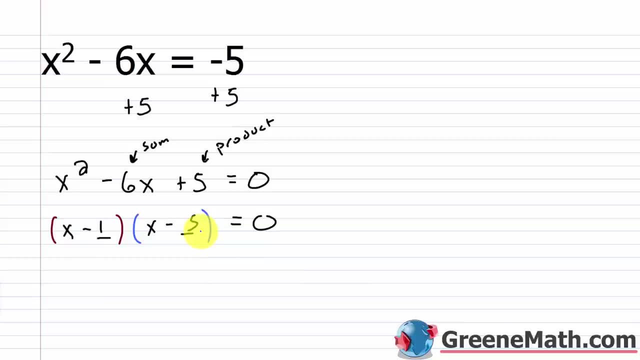 that x minus 5, that quantity is also a factor, So each one of those is going to be set equal to zero. So x minus 1 is equal to zero, or x minus 5 is equal to zero. So just solve each one for x and you can do them mentally right. 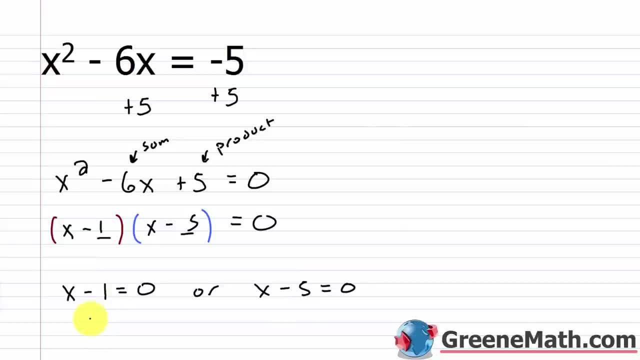 This one's going to be 1,, this one's going to be 5.. But to kind of do this for the sake of completeness, I'd add 1 to each side here. This would be: x equals 1.. I'd add 5 to each side here. 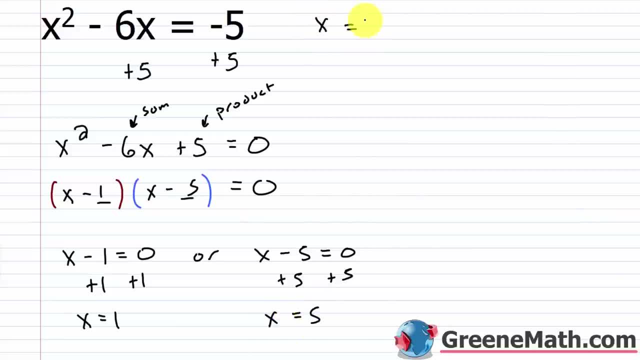 This would be x equals 1.. This would be x equals 5.. And so we get: x is equal to 1, or x is equal to 5.. So let me erase this real quick, And at this point you can just erase everything and just check in the original equation. 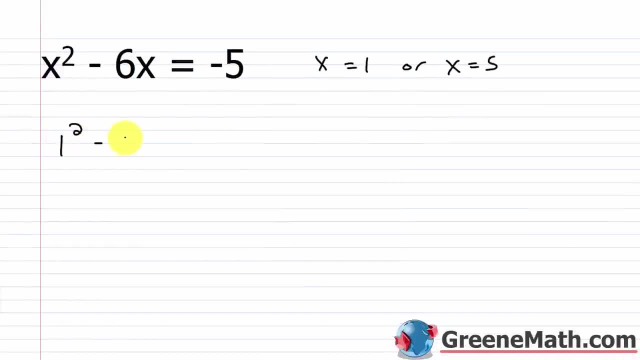 So if I plug a 1 in for x, I'd have: 1 squared minus 6 times 1 equals negative 5.. So 1 squared is 1, and then minus 6 times 1 is 6.. So 1 minus 6 is negative 5.. 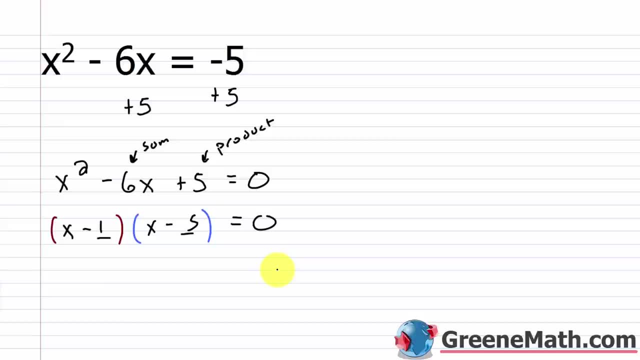 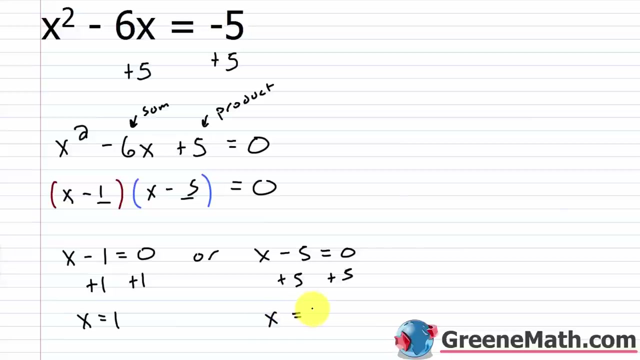 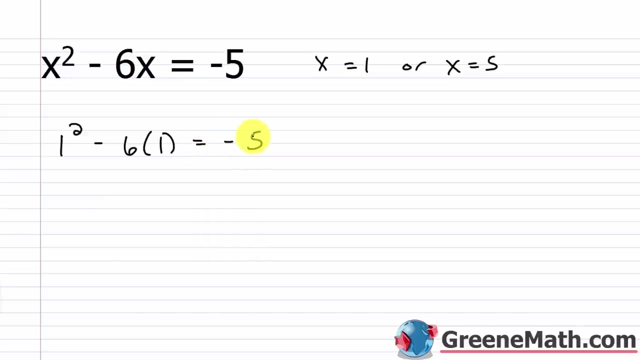 quantity is also a factor so each one of those is going to be set equal to zero so x minus one is equal to zero or x minus five is equal to zero so just solve each one for x and you can do them mentally right this one's going to be one this one's going to be five but to kind of do this for the sake of completeness i'd add one to each side here this would be x equals one i'd add five to each side here this would be x equals five and so we get x is equal to one or x is equal to five so let me erase this real quick at this point you can just erase everything and just check in the original equation so if i plug a one in for x i'd have one squared minus six times one equals negative five so one squared is one and then minus six times one is six so one minus six is negative five so negative five equals negative five so yeah this one works out then for the next one i'm plugging in a five for x so let's erase all this so i'm plugging in a five here and also here five squared is 25 minus 6 times 5 is 30 this equals negative five 25 minus 30 is negative five so negative 5 equals negative 5 so that works out as well so we can say here that x equals one or x equals five and again if you wanted to use the solution set notation you could put one comma five and show your solution that way 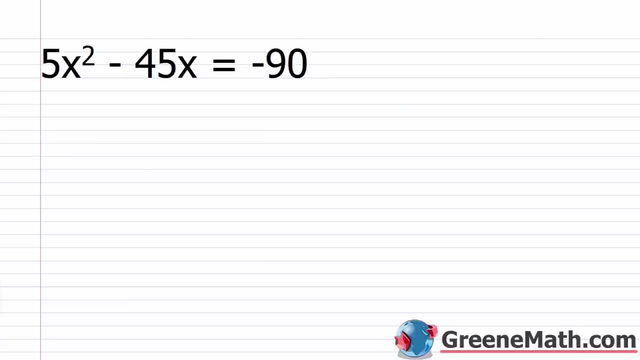 all right so what if we had something like 5x squared minus 45 x equals negative 90. well the first thing i want to do again is write this left side right and you would get umm five squared minus 45 x supervising isreal is equal five here minus km is equal negative five so that's seven мойaiek Louise and some others in standard form. So ax squared plus bx plus c. So my constant term is on the right side. I want to move this over here. So just add 90 to both sides of the equation. So I'm going to add 90 here and here. So that's going to give me 5x squared minus 45x plus 90. And remember, it's equal to zero. Negative 90 plus 90 is zero. So then I notice that everything here is divisible by five. So I want to pull that out before I even start. So if I pull that out, I'd have x squared minus 9x plus 18. Okay, so this equals zero. And I'm just going to factor what's inside, right? This trinomial in here. So I'll put the five times. I'll have two sets of parentheses. 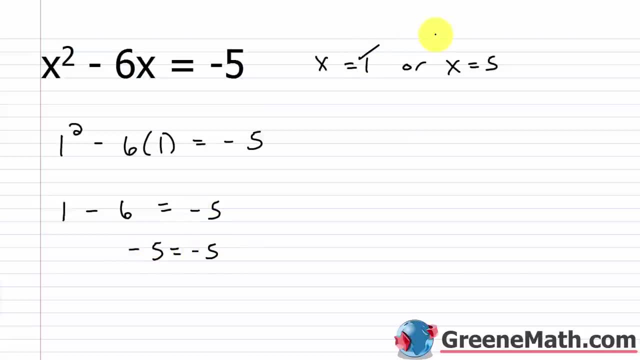 So negative 5 equals negative 5.. So, yeah, this one works out. Then for the next one, I'm plugging in a 5 for x. So let's erase all this. So I'm plugging in a 5 here and also here. 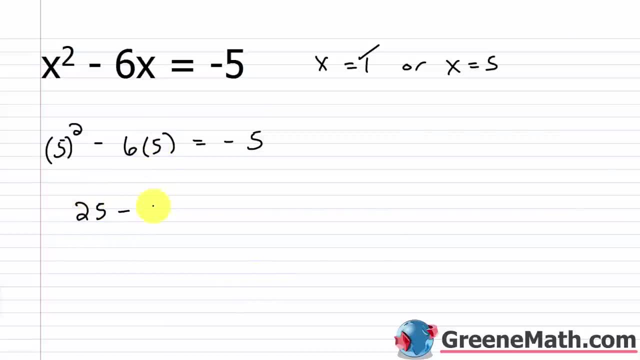 5 squared is 25 minus 6 times 5 is 30.. This equals negative 5.. 25 minus 30 is negative 5.. So negative 5 equals negative 5. So that works out as well. So we can say here that x equals 1 or x equals 5.. 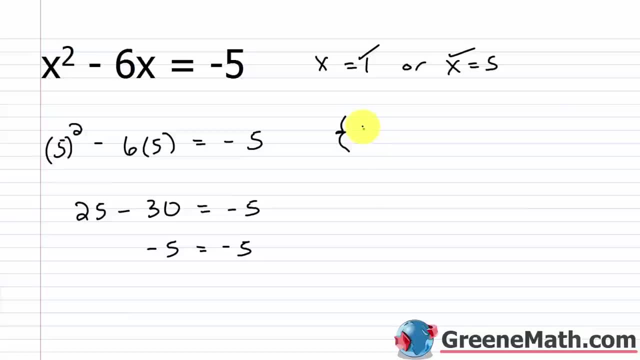 And again, if you wanted to use the solution set notation, you could put 1 comma 5 and show your solution that way. All right, So what if we had something like: 5x squared minus 45x equals negative 90?? 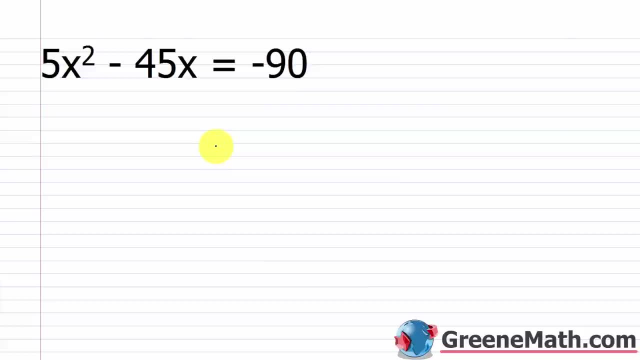 Well, the first thing I want to do again is write this left side in standard form, So ax squared plus bx plus c. So my constant term is on the right side. I want to move this over here. So just add 90 to both sides of the equation. 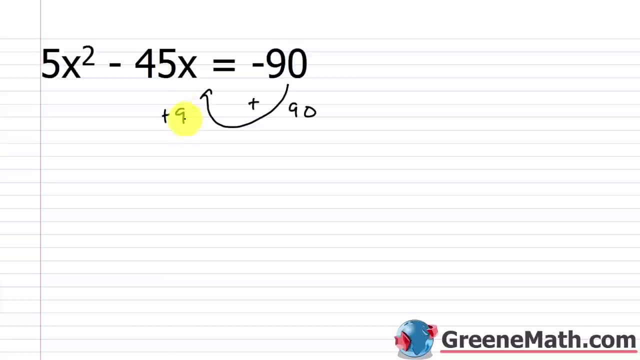 So I'm going to add 90 here and here. So that's going to give me 5x squared minus 45x plus 90.. And then, remember, it's equal to 0.. Negative 90 plus 90 is 0.. 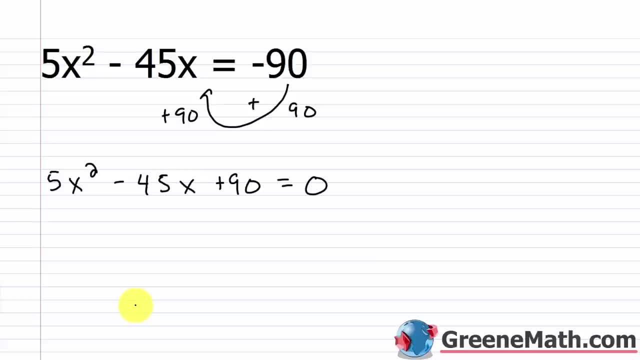 So then I notice that everything here is divisible by 5. So I want to pull that out before I even start. So if I pull that out, I'd have x squared minus 9x plus 18.. OK, so this equals 0.. 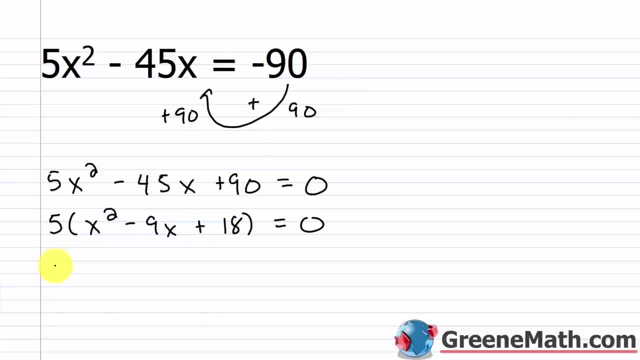 And I'm just going to factor what's inside right This trinomial in here. So I'll put the 5. Times, I'll have two sets of parentheses And this equals 0.. So I know this is x and this is x. 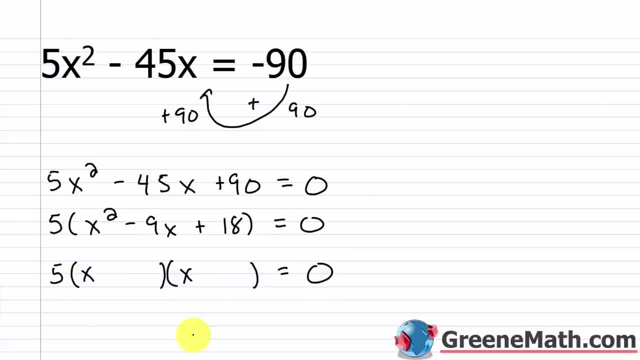 So give me two integers whose sum is negative 9 and whose product is 18.. So if I think about the factors of 18, you think about negative 6 and negative 3, right? Negative 6 plus negative 3 is negative 9.. 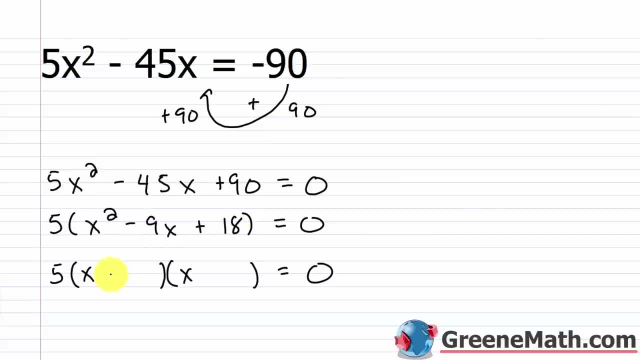 Negative 6 times negative, 3 is 18.. So minus 6 and then minus 3.. So once we have that, we can solve this. Take each factor and set it equal to 0.. Now 5 is a factor here. 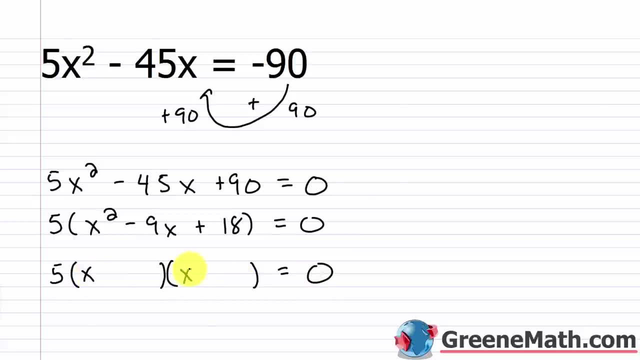 And this equals zero. So I know this is x and this is x. So give me two integers whose sum is negative nine and whose product is 18. 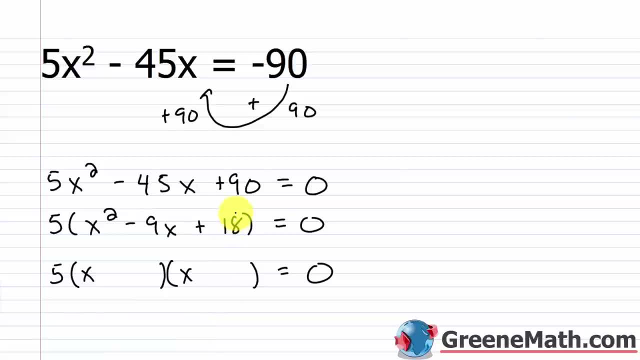 So if I think about the factors of 18, you think about negative six and negative three, right? Negative six plus negative three is negative nine. Negative six times negative 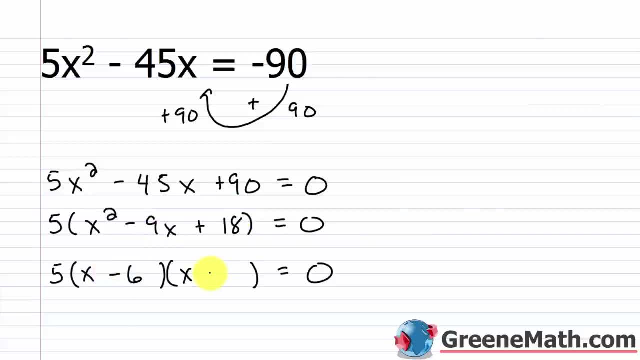 three is 18. So minus six and then minus three. So once we have that, we can solve this. 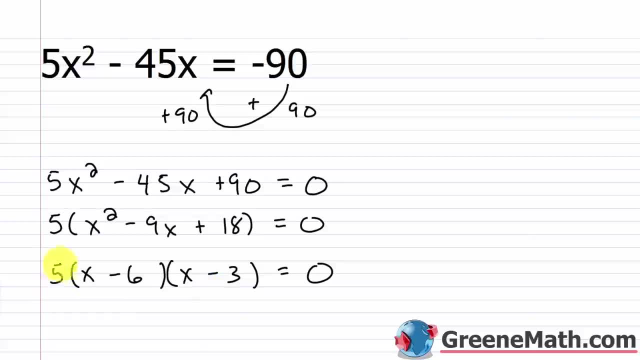 Take each factor and set it equal to zero. Now, five is a factor here, but there's no variable involved. Five doesn't equal zero. So it wouldn't make any sense for me to say, okay, this factor five equals zero. So 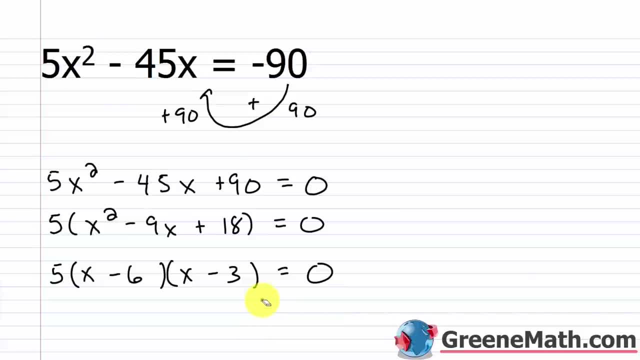 you can kind of modify that and say that you want to set each factor with a variable equal to zero. So then I would take x minus six and set that equal to zero. And then or we'd have x minus three equals zero. Let me scroll down a little bit. And obviously we can eyeball that and 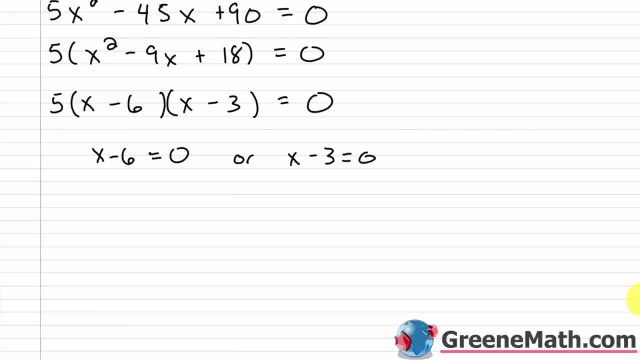 say x can be six or x can be three, right? But again, for the sake of completeness, add six to both sides of the equation. That gives you x equals six. Add three to both sides of the equation. That gives you x equals six. And then I would take x minus six and set that equal to zero. And then 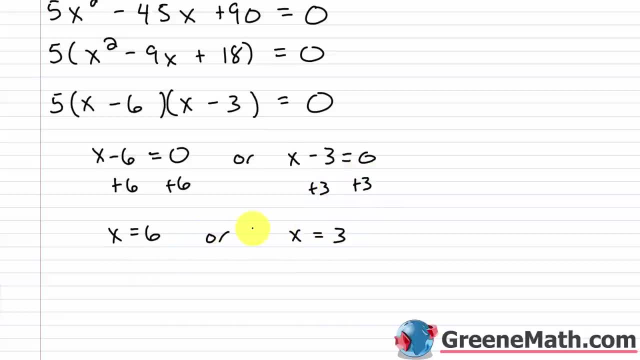 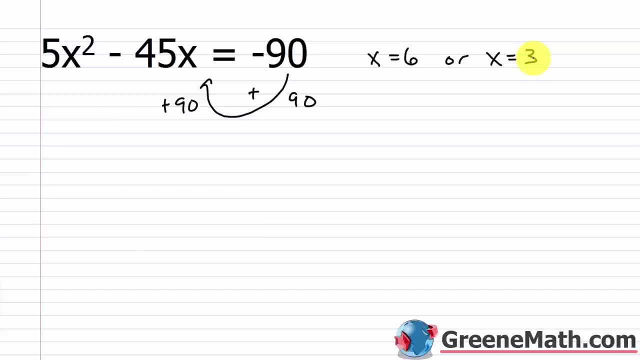 we get x equals three. So we get x equals six or x equals three. So then again, x equals six or x equals three. All right, so let's check this in the original equation. So I'd have five times 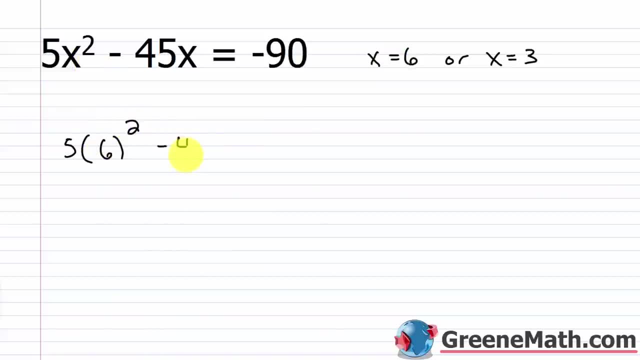 plug in a six for x. That's squared minus 45 times plug in a six for x. This equals negative 90. So six squared is 36. So I'd have five times 36, which is 180. Minus 45 times six, which is 270. This should equal negative 90. And it does, right? You get negative 90 equals negative 90. So this one checks out. And then for x equals three, let's erase all 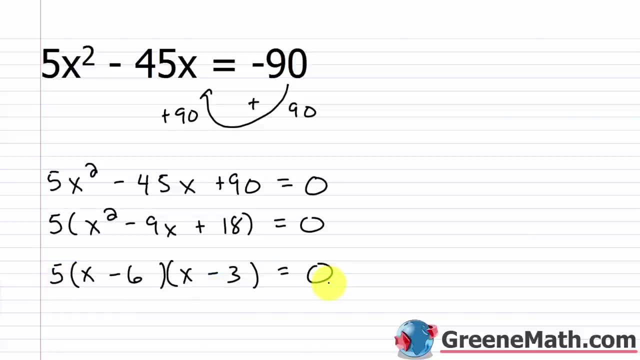 But there's no variable involved. 5 doesn't equal 0. So it wouldn't make any sense for me to say, OK, this factor of 5 equals 0. So you can kind of modify that and say that you want to set each factor with a variable equal to 0. 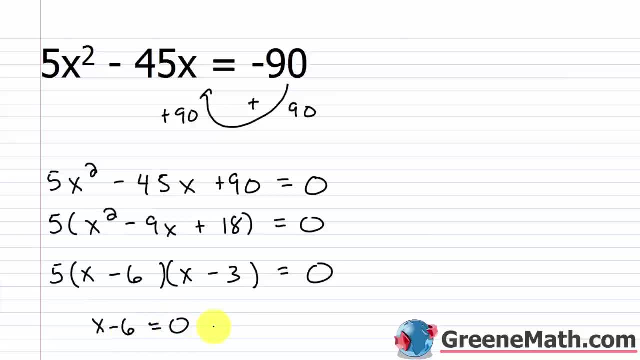 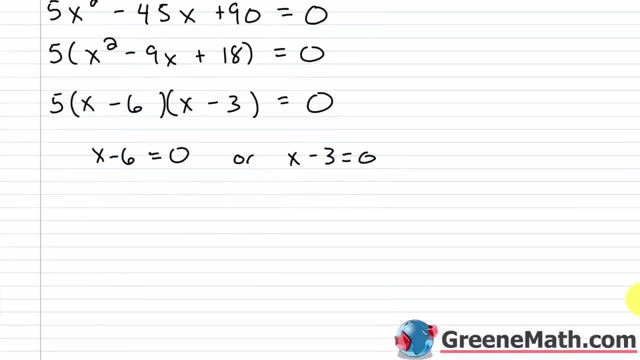 So then I would take x minus 6 and set that equal to 0. And then or we'd have x minus 3 equals 0. Let me scroll down a little bit, And obviously we can eyeball that and say: 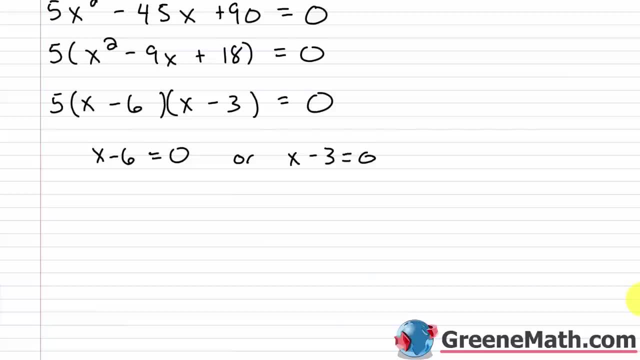 x can be 6 or x can be 3, right, But again, for the sake of completeness, add 6 to both sides of the equation. That gives you x equals 6.. Add 3 to both sides of the equation. 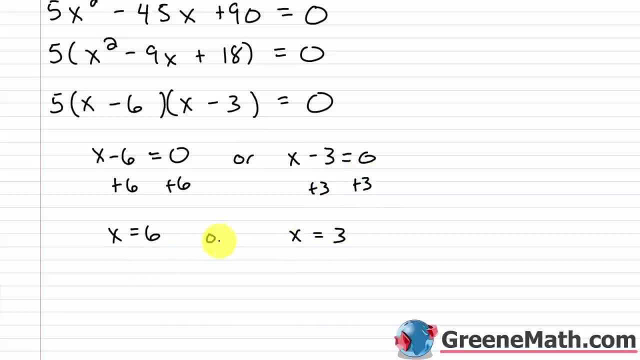 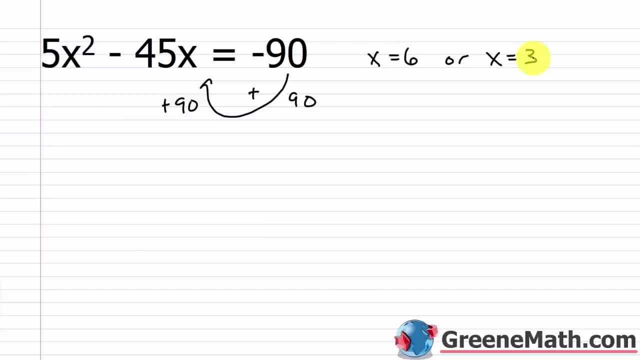 That gives you x equals 3.. So we get x equals 6 or x equals 3.. So then again, x equals 6 or x equals 3.. All right, so let's check this in the original equation. So I'd have 5 times plug in a 6 for x. 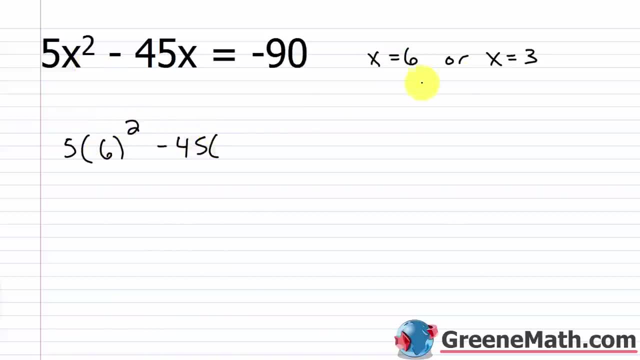 That's squared minus 45 times plug in a 6 for x, This equals negative 90. So 6 squared is 36.. So I'd have 5 times 36,, which is 180, minus 45 times 6,, which is 270.. 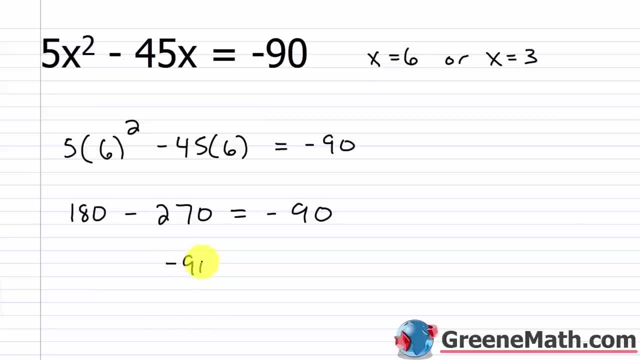 This should equal negative 90. And it does You get. negative 90 equals negative 90. So this one checks out. And then for x equals 3.. Let's erase all this. Put a 3 here, and here 3 squared is 9.. 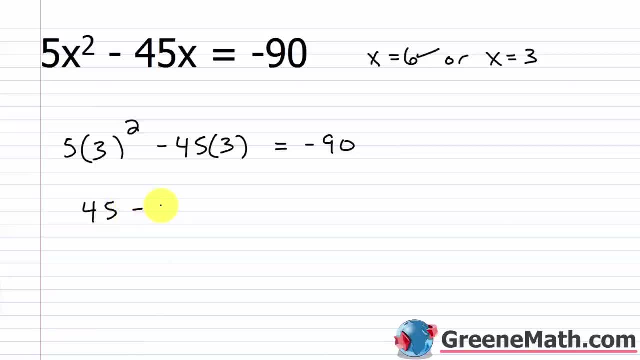 9 times 5 is 45. And then minus 45 times 3, which is 135. And this should equal negative 90. And again it does, You get: negative 90 equals negative 90. So this works as a solution as well. 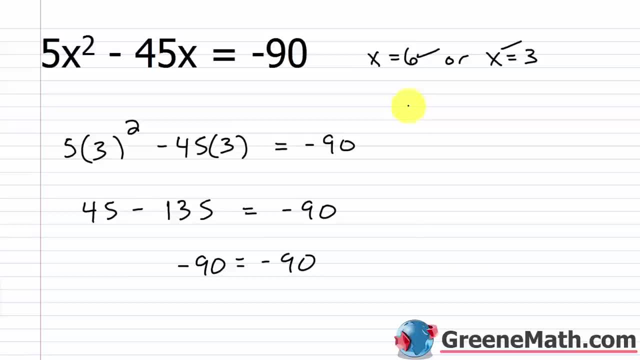 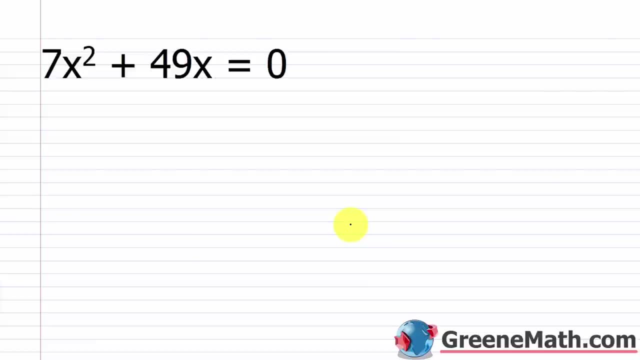 So x equals 6 or x equals 3.. Again you could write this like this as 3 comma 6 in your solution set notation. All right, let's take a look at another one. Let's say you had 7x squared plus 49.. 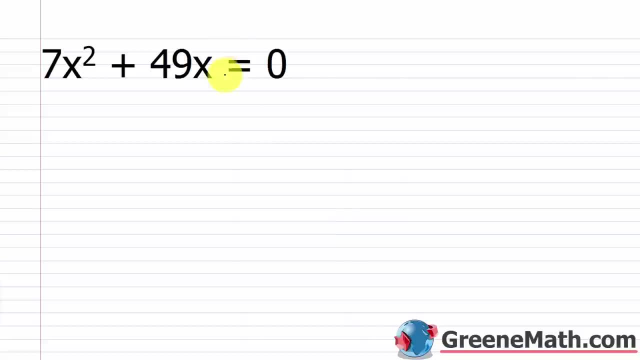 7x equals 0. So it looks like I'm missing a constant over here. I could put plus 0 there, but really that's just the same thing, right? So is there a way to factor this? Well, the answer is yes. 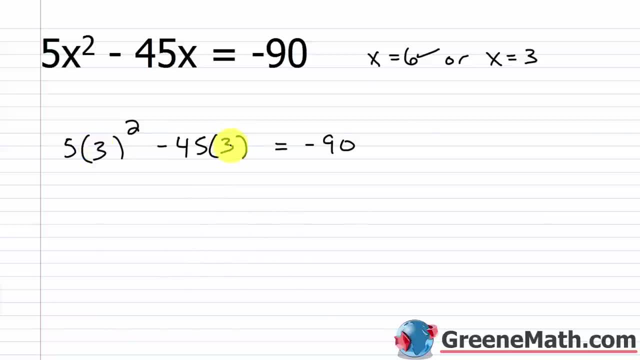 this. Put a three here and here. Three squared is nine. Nine times five is 45. And then minus 45 times three, which is 135. And this should equal negative 90. And again, it does. You get negative 90 equals negative 90. And then for x equals three, let's erase all this. Put a three here and here. 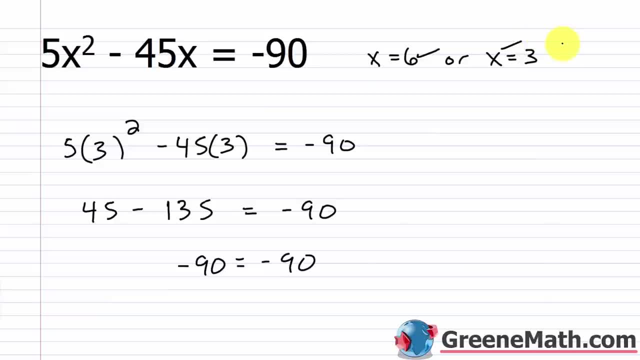 Negative 90. So this works as a solution as well. So x equals six or x equals three. Again, you could write this like this as three comma six in your solution set notation. All right, 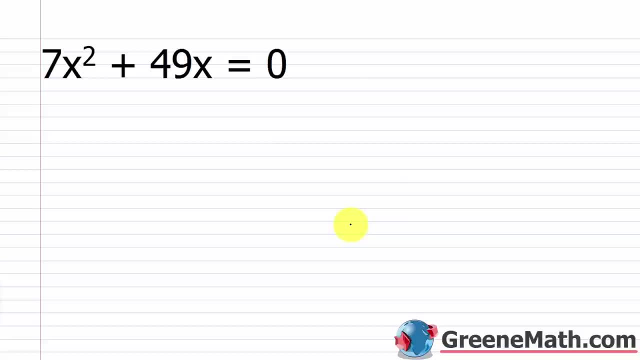 let's take a look at another one. Let's say you had seven x squared plus 49 x equals zero. So it looks like I'm missing a constant over here. I could put plus zero there, but really that's just the same thing, right? So is there a way to factor this? Well, the answer is yes. Each term here is divisible by seven x. So I can pull that out. So I could say I have seven x times inside of parentheses. If I divided this by seven x, I just have x. Plus if I divided this by seven x, I just have seven. And this equals zero. Well, I have two factors here that are equal to zero. 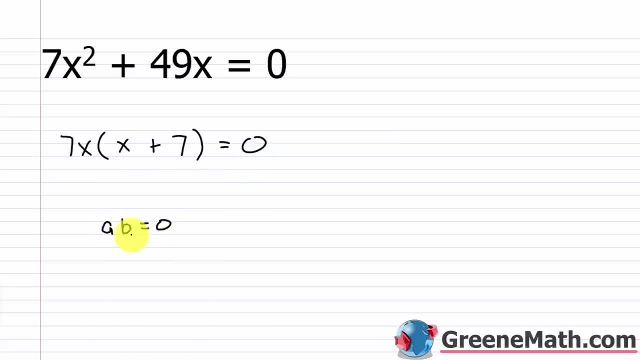 Remember, my original is a b equals zero. If that occurs, then a equals zero, b equals zero, or both a and b equal zero. 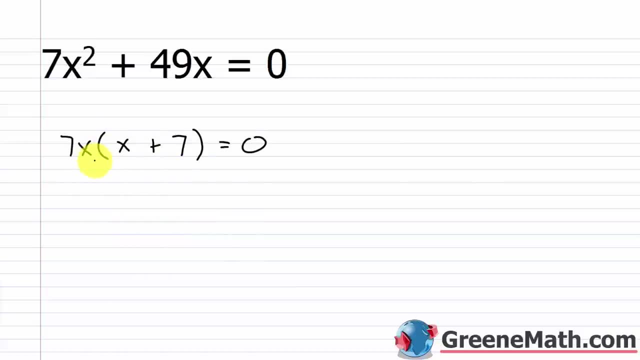 So I can set each factor here because they each have a variable involved equal to zero and I can solve. So I could say seven x equals zero or x plus seven equals zero. Now, seven x equals zero is very straightforward. You divide both by seven and you get x equals zero. So x can be zero or if we have x plus seven equals zero, subtract seven away from each side of the equation, you get x equals negative seven. So or, 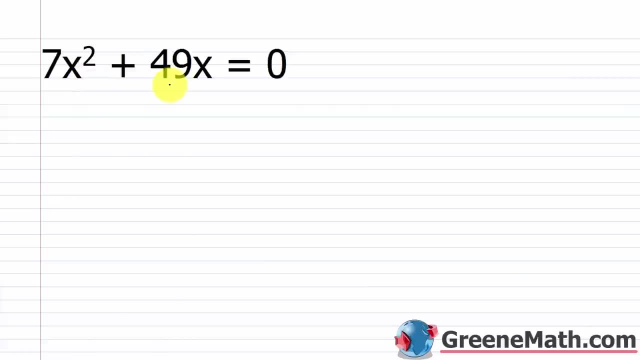 Each term here is divisible by 7x, So I can pull that out. So I could say I have 7x times inside of parentheses. If I divided this by 7x, I just have x plus. if I divided this by 7x, I just have 7.. 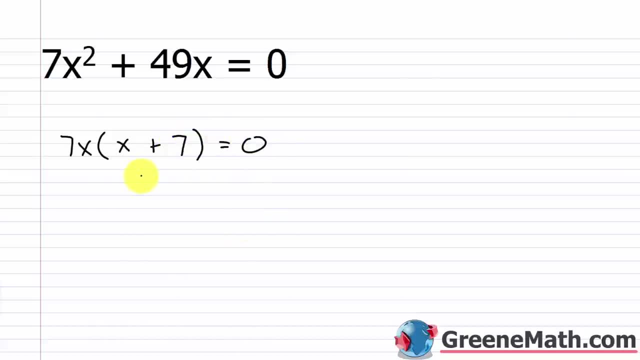 This equals 0.. Well, I have two factors here that are equal to 0.. Remember, my original is: a, b equals 0. If that occurs, then a equals 0,, b equals 0, or both a and b equal 0. 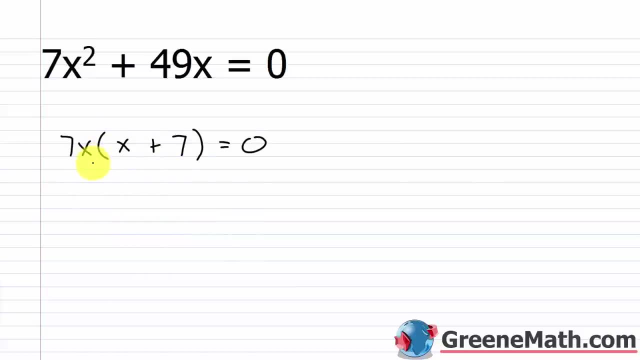 So I can set each factor here, because they each have a variable involved equal to 0, and I can solve. So I could say 7x equals 0, or x plus 7 equals 0. Now 7x equals 0 is very straightforward. 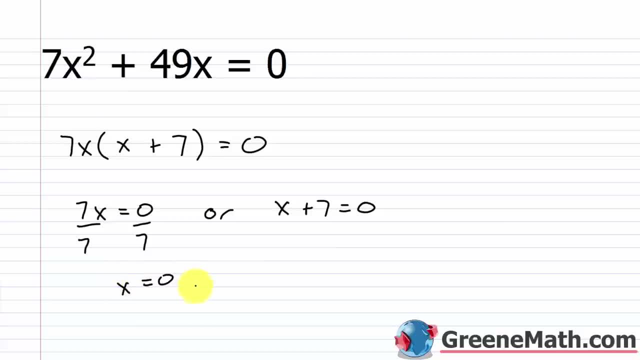 You divide both by 7, and you get x equals 0. So x can be 0, or if we have x plus 7 equals 0, subtract 7 away from each side of the equation, you get x equals negative 7.. 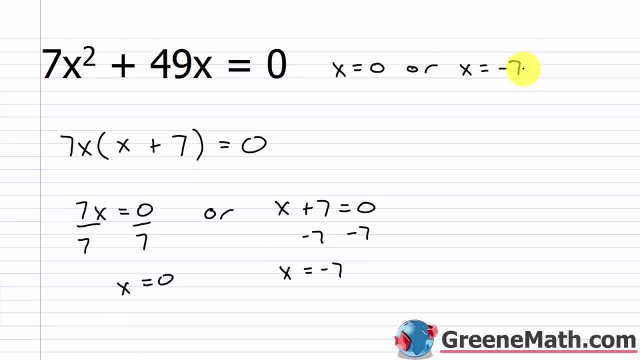 So or x equals negative 7.. So let's check both of these. Obviously, 0 works. If I plug a 0 in here, I'd get 0 times 7, that's 0.. Plug a 0 in here, I'd get 0.. 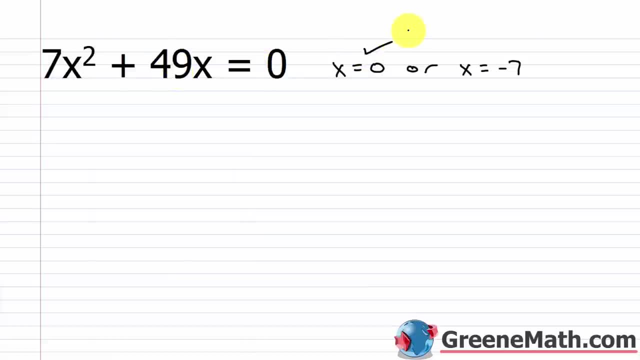 0 plus 0 is 0.. That works out For negative 7, you'd have 7 times the quantity negative 7 squared. Remember, if I'm plugging in something for x and it's being squared, I want what's being plugged in squared. 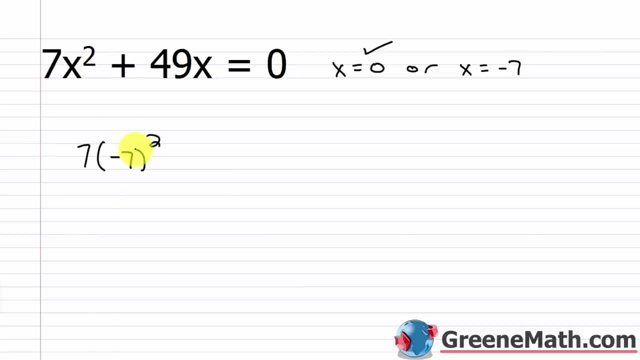 So negative 7 is being plugged in, so I've got to use parentheses to say I want both the negative and the 7 to be squared. So then plus 49 times negative 7. And then this equals 0.. And so what are we going to get here? 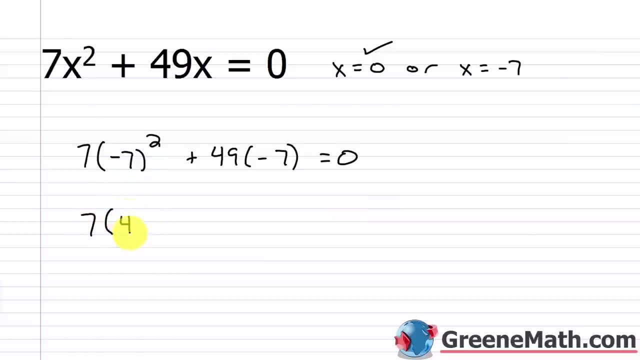 Well, negative 7 squared is 49. So you'd have 7 times 49 plus 49 times negative. 7 equals 0. You don't even need to do the multiplication because these two numbers would be opposites. I have positive times positive and I have negative times positive. 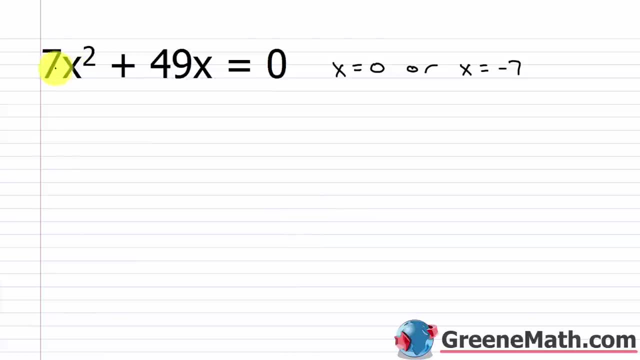 Obviously, zero works. If I plug a zero in here, I'd get zero times seven, that's zero. Plug a zero in here, I'd get zero. Zero plus zero is zero. That works out. For negative seven, you'd have seven times the quantity negative seven squared. Remember, if I'm plugging in something for x and it's being squared, I want what's being plugged in to be zero. So I can plug a zero in here, I'm plugging in something for x and it's being squared. So negative seven is being plugged in. So I've got to use parentheses to say I want both the negative and the seven to be squared. So then plus 49 times negative seven. And then this equals zero. And so what are we going to get here? Well, negative seven squared is 49. So you'd have seven times 49 plus 49 times negative seven equals zero. You don't even need to do the multiplication because 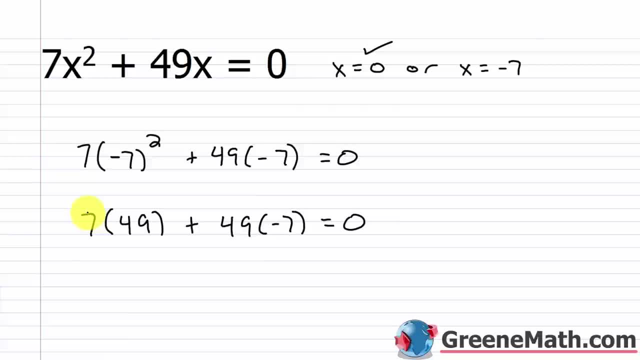 these two numbers would be opposites. I have positive times positive, and I have negative. times positive. So this would be negative, this would be positive, it would be the same number, they would just be opposites. This would be positive 343, and this would be negative 343. 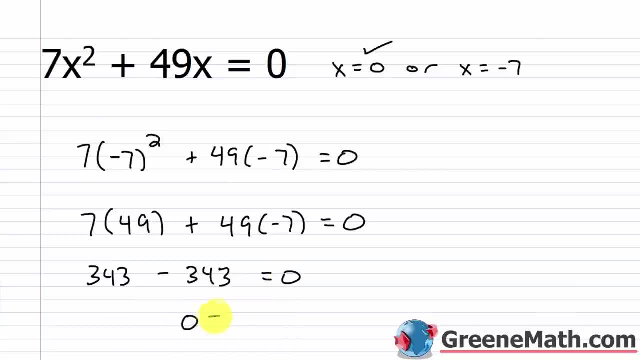 So you'd have 343 minus 343 equals zero. So zero equals zero. So yes, x equals negative seven is a solution. So you get x equals zero or x equals negative seven. Again, you could write that using solution set notation as negative seven comma zero inside the set braces. 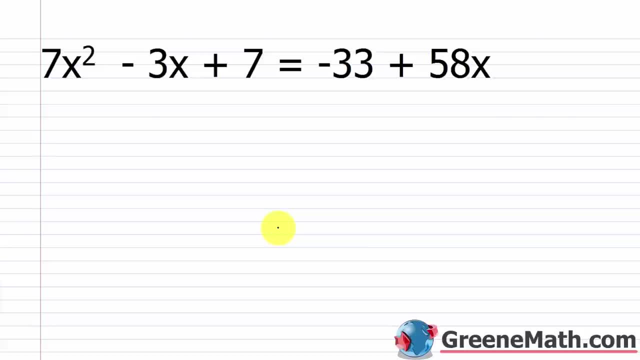 So let's look at a harder one. We have 7x squared minus 3x plus 7. This is equal to negative 33 plus 58x. So we're going to add 33 to both sides of the equation. 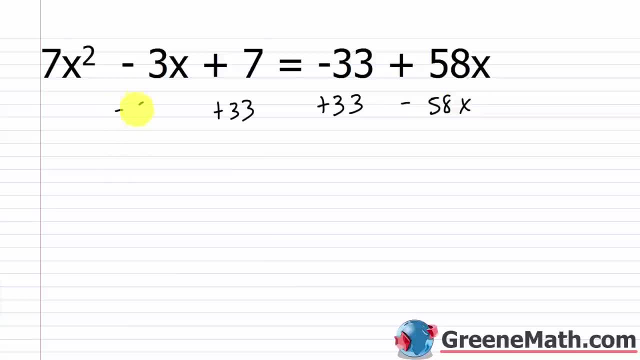 Then we're going to subtract 58x from both sides of the equation. And so let's cross this out and this out and put this together. So we're going to add this out and this out. So we're going to add this out and this out and put this out and put this out and put this out. 0. And then over on the left hand side, we'll have 7x squared. Negative 3x minus 58x is going 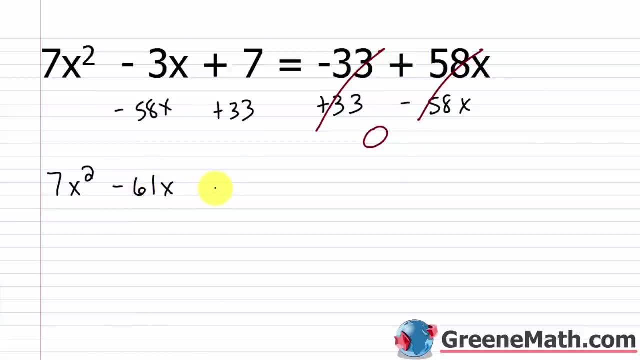 to be negative 61x. And then 33 plus 7 is 40. So plus 40. And this equals 0. So let's go ahead and factor the left side. Now we have one where the a the coefficient of the x squared term is 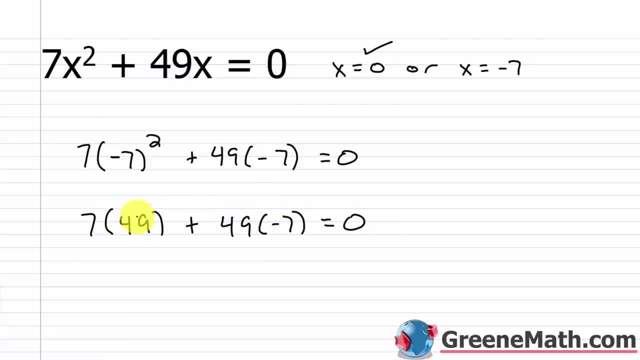 So this would be negative. This would be positive, It would be the same number, It would just be opposites. This would be positive, 343, and this would be negative 343.. So you'd have 343 minus 343 equals 0.. 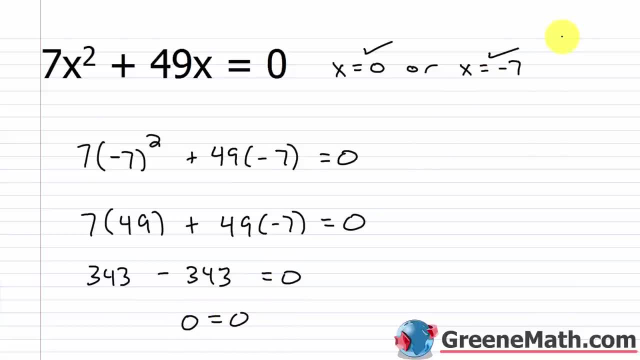 So 0 equals 0. So yes, This equals negative 7 is a solution. So you get x equals 0 or x equals negative 7.. Again, you could write that using solution set notation as negative 7, comma 0, inside the set braces. 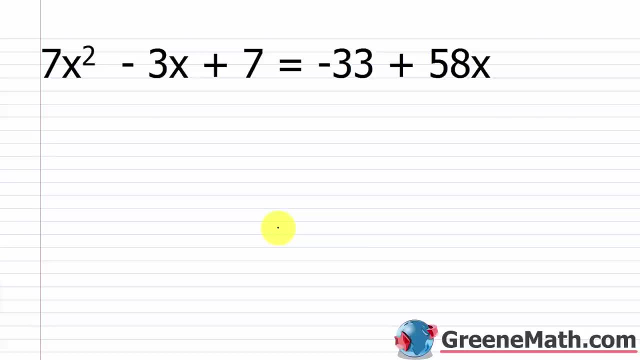 So let's look at a harder one. We have 7x squared minus 3x plus 7. This is equal to negative 33 plus 58x. So we're going to add 33 to both sides of the equation And then we're going to subtract. 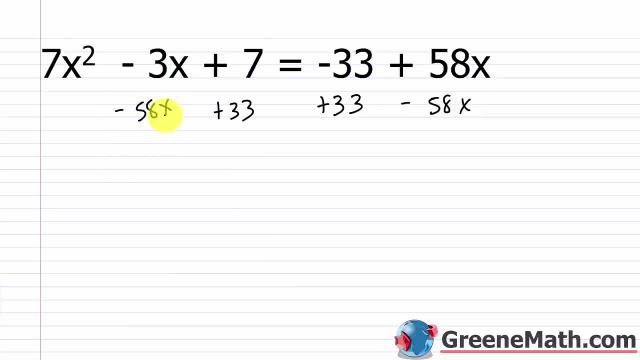 We're going to subtract 58x from both sides of the equation, And so let's cross this out and this out and put a 0. And then, over on the left-hand side, we'll have 7x squared. Negative 3x. minus 58x is going to be negative 61x. 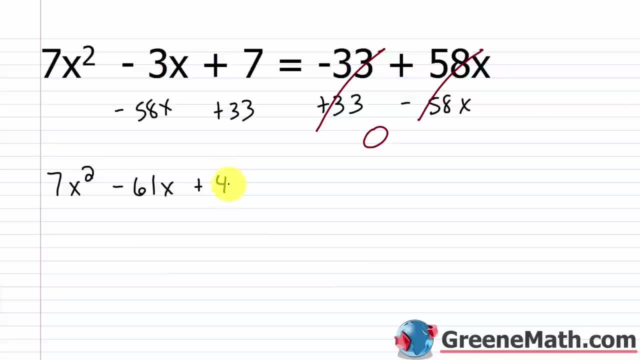 And then 33 plus 7 is 40. So plus 40. And this equals 0.. So let's go ahead and factor the left side. Now we have one where the a, the coefficient of the x squared term, is not 1.. 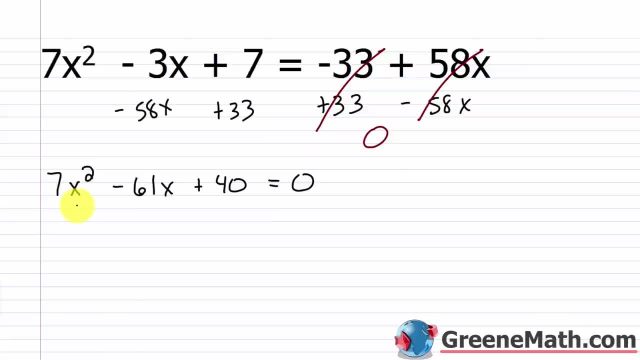 So this requires a little bit more work to factor, But that's OK, We already learned how to do that in a previous lesson, Remember. what I'm going to do is I'm going to take two integers. whose product is this times this? 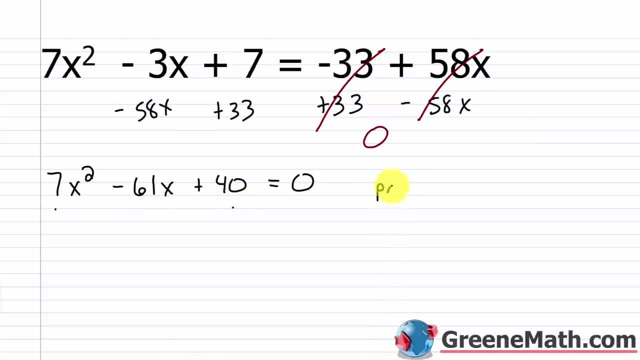 So 7 times 40, which would be 280.. So product of 280 and whose sum is negative, 61, right The b, the coefficient for the x to the first power term, So sum of negative 61.. So let's think about some factors of 280.. 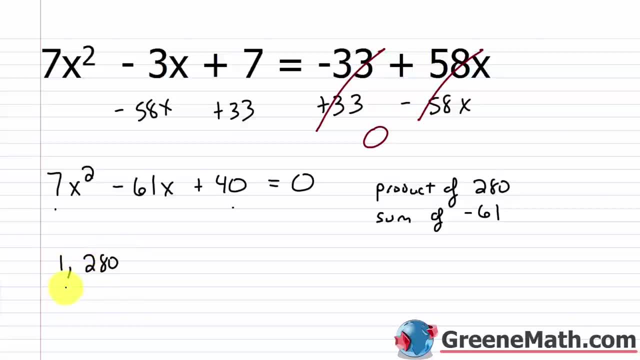 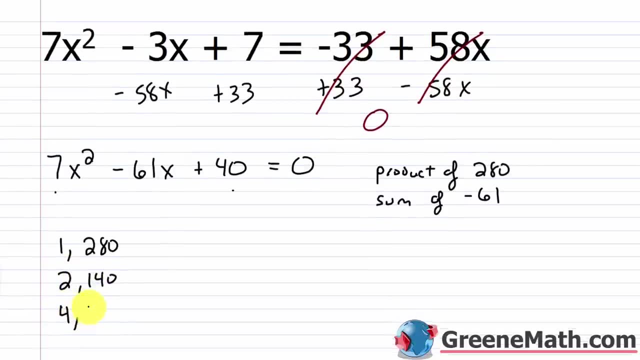 We have 1 times 280.. That's not going to work. We have 2 times 140. That's obviously not going to work. Not divisible by 3. You could do 4 times 70. That's not going to really work. 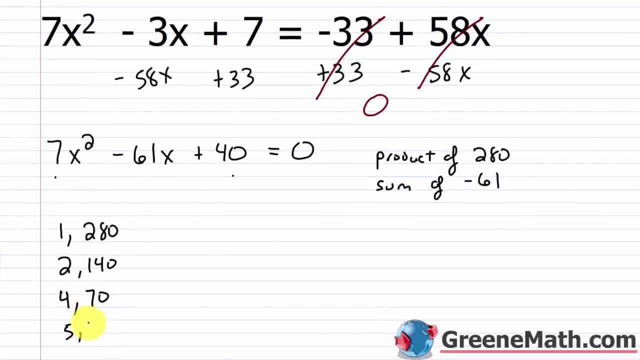 And then you could do 5 times 56.. Now we could play with the signs and make that work. The product is positive, but the sum is negative, So all I need to do is have 2.. Negative 5 plus negative 56 is negative 61.. 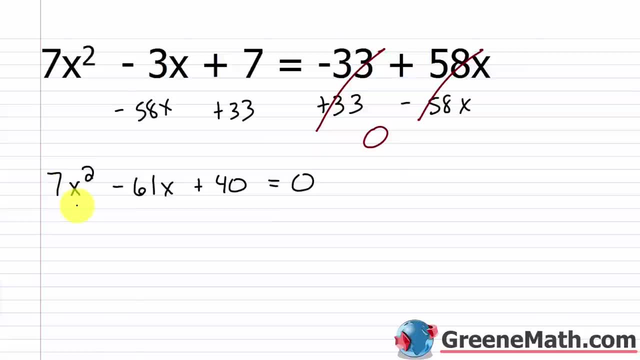 not one. So this requires a little bit more work to factor. But that's okay, we already learned how to do that in a previous lesson. Remember, what I'm going to do is I'm going to take two integers, whose product is this times this. So seven times 40, which would be 280. So product of 280. And whose sum is negative 61, right, the B, the coefficient for the x to the first power term. So sum of negative 61. So let's think about some factors of 280. 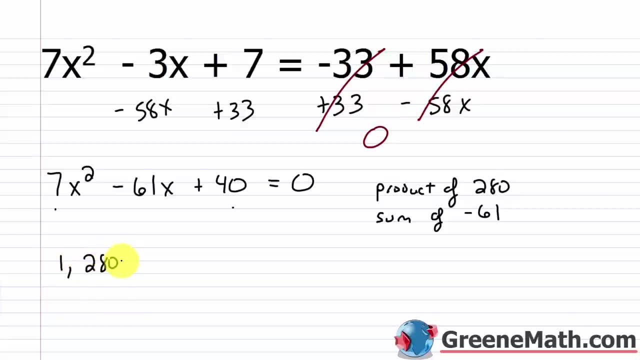 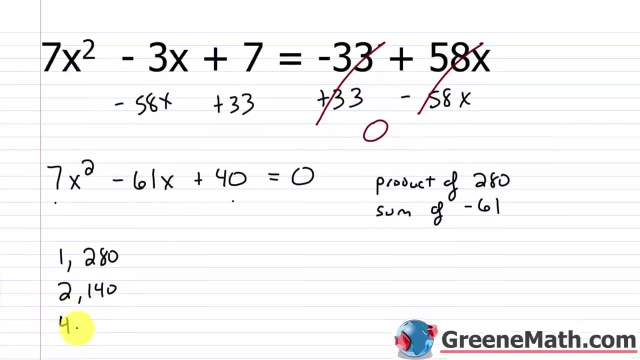 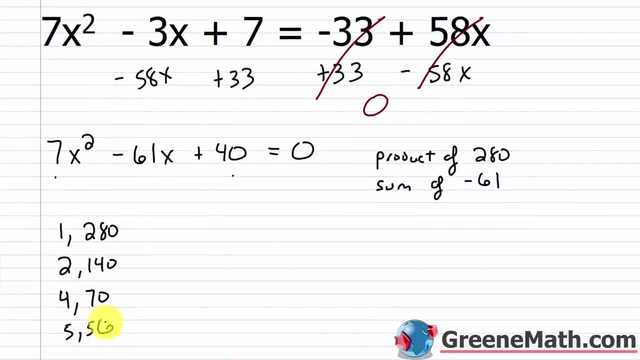 We have one times 280. That's not going to work. We have two times 140. It's obviously not going to work. Not divisible by three, you could do four times 70. That's not going to really work. And then you could do five times 56. Now we could play with the signs and make that work. The product is positive, but the sum is negative. So all I need to do is have two negative signs. Negative five plus negative 56 is negative 61. Negative five times, negative 56 is 280. So that will work. Five and 56. All I'm going to do is use that to rewrite that middle term. So I'm going to have seven x squared, I'm going to put minus 56 x, then I'm going to put minus five x plus 40 equals zero. And now I'm going to factor using grouping. 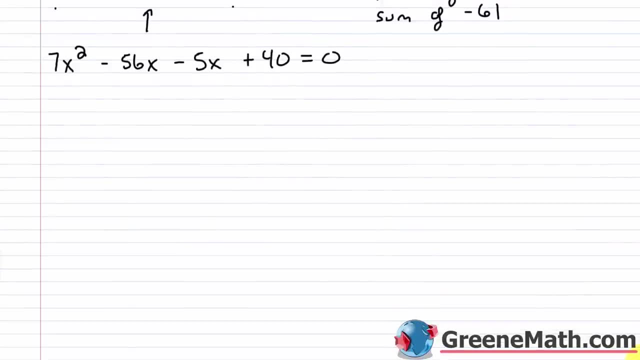 Let's scroll down a little bit. So out of this first group, the seven x squared minus 56 x, I can pull out a seven x. 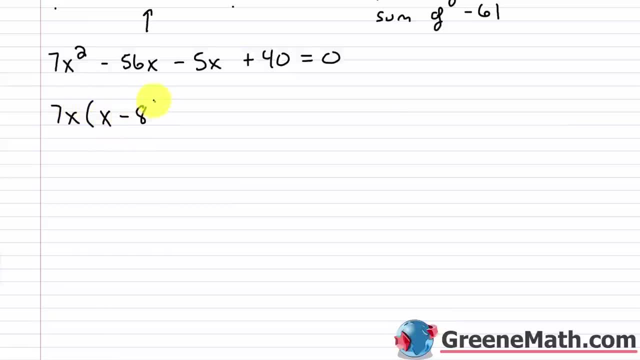 So that's going to be negative 56 x minus 56 x. That would leave me with x minus eight. Out of the second group, I can pull out a negative five and be left with an x minus eight. This equals zero. Obviously, the common binomial factor is x minus eight. So I'll have seven x minus five, that quantity, times x minus eight, that quantity. 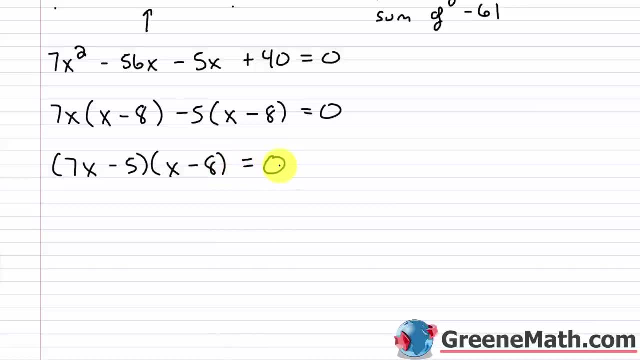 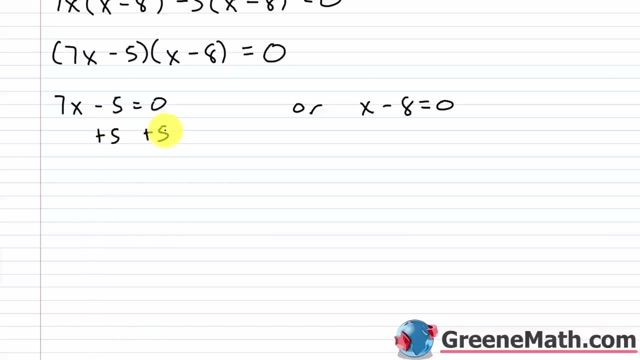 This is going to be equal to zero. So now all I need to do is set each of these factors equal to zero, and I'll have my answer. So seven x, minus five equals zero, or x minus eight equals zero. So for this one, I just need to add five to both sides of the equation. I'll have seven x is equal to five, divide both sides of the equation by seven, x equals five sevenths. For this one, I'll add eight to both sides of the equation, and I'll have x is equal to eight. So x equals five sevenths, or x equals eight. 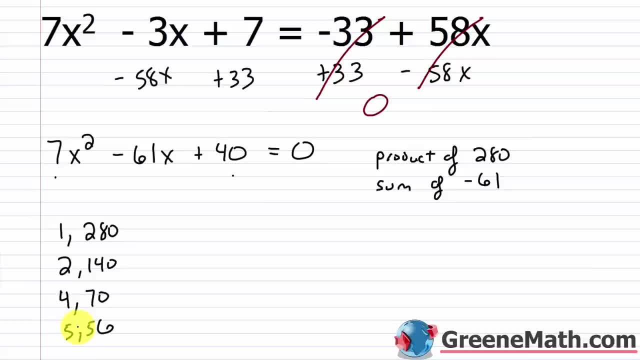 Negative 5 times negative, 56 is 280.. So that will work: 5 and 56.. All I'm going to do is use that to rewrite that middle term. So I'm going to have 7x squared. I'm going to put minus 56x. 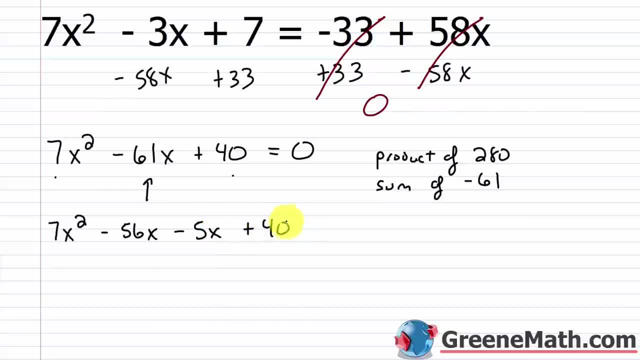 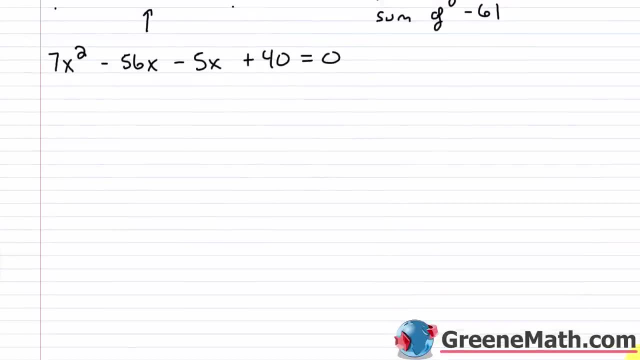 Then I'm going to put: minus 5x plus 40 equals 0.. And now I'm going to factor using grouping. Let's scroll down a little bit. So out of this first group, the 7x squared minus 56x. 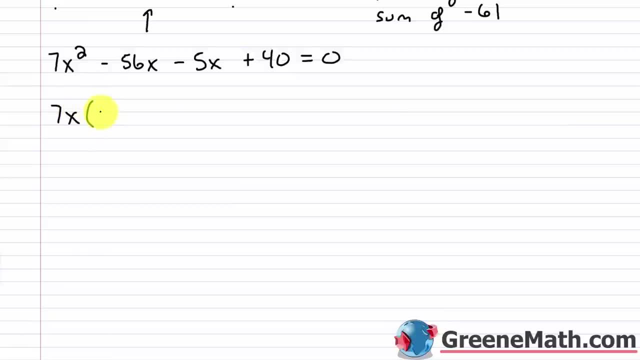 I can pull out a 7x, So that would leave me with x minus 8.. Out of the second group I can pull out a negative 5 and be left with an x minus 8. This equals 0. Obviously, the common binomial factor is x minus 8.. 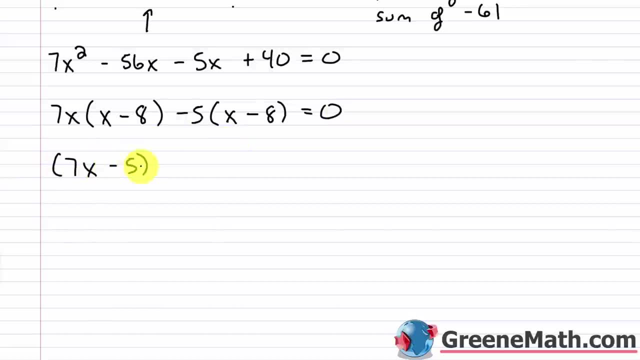 So I'll have 7x minus 5, that quantity times x minus 8, that quantity, This is going to be equal to 0.. So Now all I need to do is set each of these factors equal to 0 and I'll have my answer. 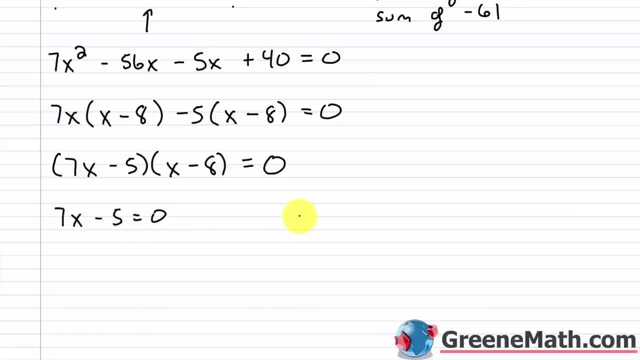 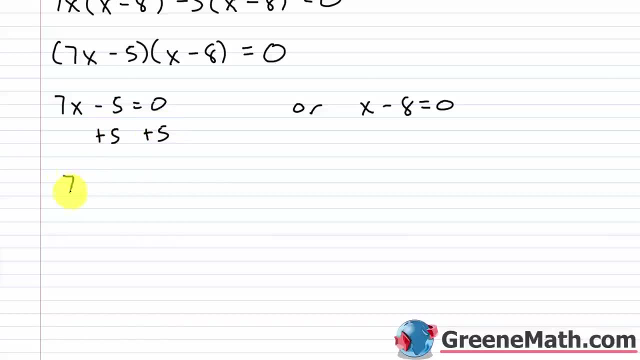 So 7x minus 5 equals 0, or x minus 8 equals 0. So for this one I just need to add 5 to both sides of the equation. I'll have 7x is equal to 5.. Divide both sides of the equation by 7.. 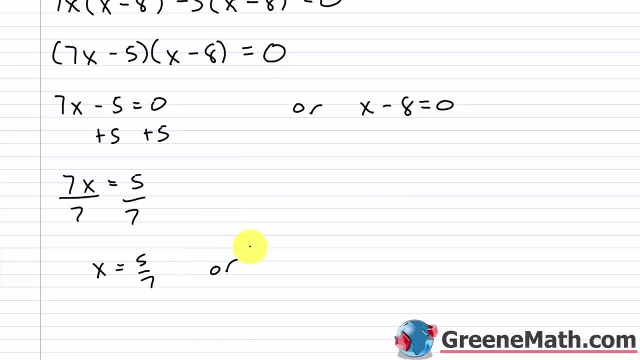 x equals 5 sevenths. For this one, I'll add 8 to both sides of the equation and I'll have: x is equal to 8.. So x equals 5 sevenths Or x equals 8.. All right, so let's check these two proposed solutions. 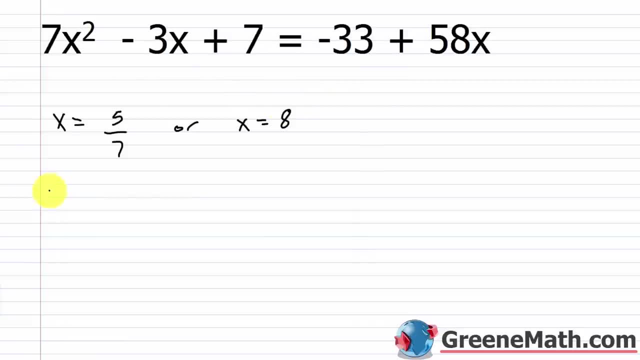 So the first one is a little bit more tedious, So let's go ahead and get that out of the way. So we have 7 times 5 sevenths squared, minus 3 times 5 sevenths. plus 7 equals negative 33 plus 58 times 5 sevenths. 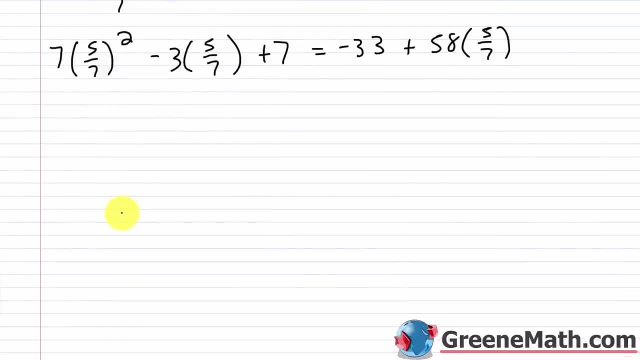 So let's work through this guy. So 5 sevenths squared would be 25 forty-ninths, So you'd have 7 times, So you'd have 7 times, So you'd have 7 times 25 over 49.. 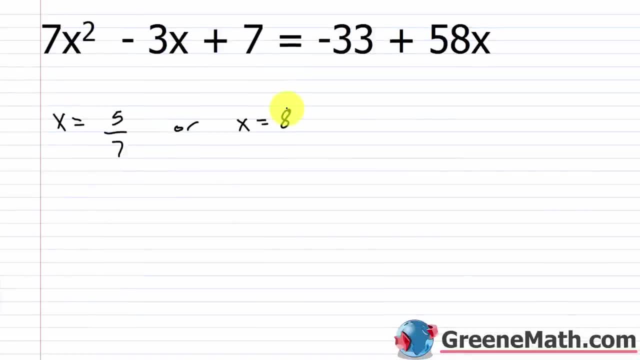 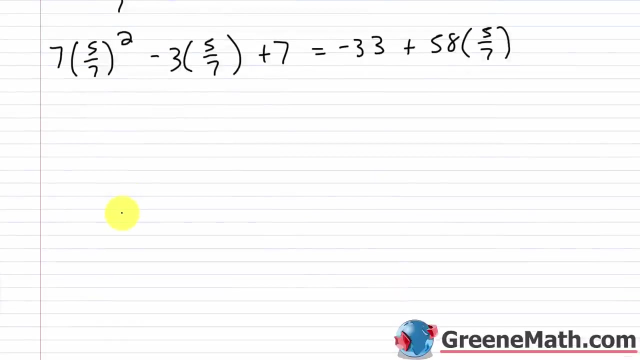 All right, so let's check these two proposed solutions. Well, the first one is a little bit more tedious. So let's go ahead and get that out of the way. So we have seven times five sevenths squared, minus three times five sevenths, plus seven equals negative 33, plus 58 times five sevenths. So let's work through this guy. So five sevenths squared would be 25 forty-ninths. So you'd have seven times 25 over 49. This would cancel with this and give me a seven down here. So 25. Five sevenths is what that would be. And then minus, you have three times five sevenths. Nothing I can really cancel there. So I'm going to write 15 sevenths, and then plus seven. Before I go on over here, let me just get a common denominator going. So I could write this as 49 over seven. And then I could just perform the operation with the numerators. 25 minus 15 is 10. 10 plus 49 is 59. So this is 59 over seven. 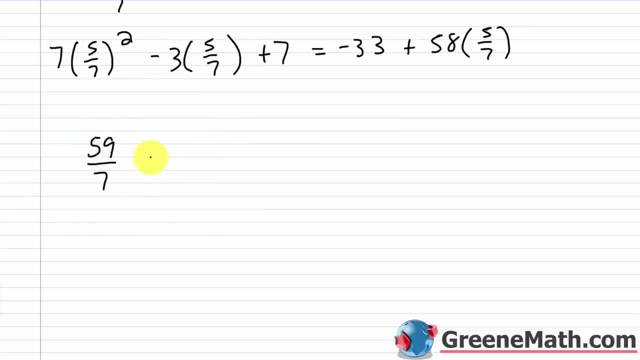 Now to avoid articles on the left side. So 59 sevenths.. And this equals over here if I do the multiplication of 58 times 5 sevenths. Well, 58 times 5 is 290. So I'd have negative 33, plus 290 over seven. Now to get a common denominator here, I'd multiply this by seven over seven, and I get negative 231. So this would be negative 231 over seven. If I do negative 231, plus 290, this would I get 59. So you'd end up with 59 7ths is equal to 59 7ths. So this one checks out. And then the 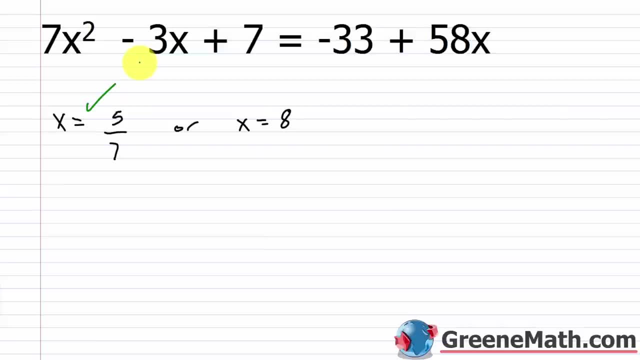 second one is that x equals 8. That one's a lot easier to do. So let's knock that out real quick. 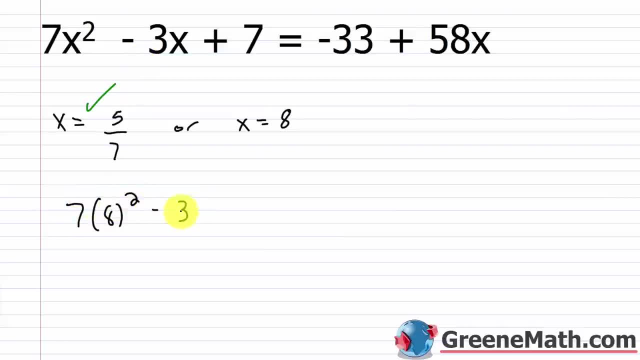 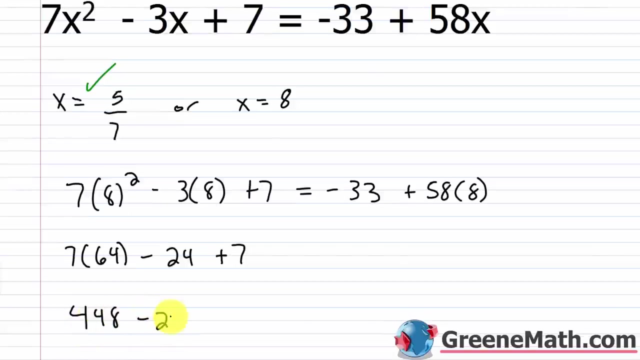 So 7 times, you'll have 8 squared minus 3 times 8 plus 7. This is equal to negative 33 plus 58 times 8. So 8 squared is what? That's 64. So 7 times 64 minus 3 times 8 is 24 plus 7. So 7 times 64 is 448. So 448 minus 24 plus 7. Over here, let's just do some of this. 58 times 8 is 464. 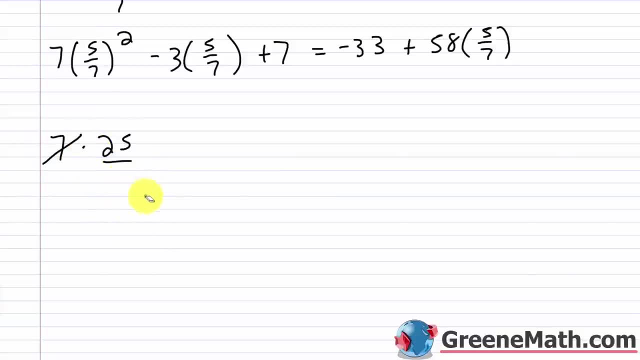 This would cancel with this and give me a 7 down here. So 25 sevenths is what that would be, And then minus you have 3 times 5 sevenths. Nothing I can really cancel there. So I'm going to write 15 sevenths. 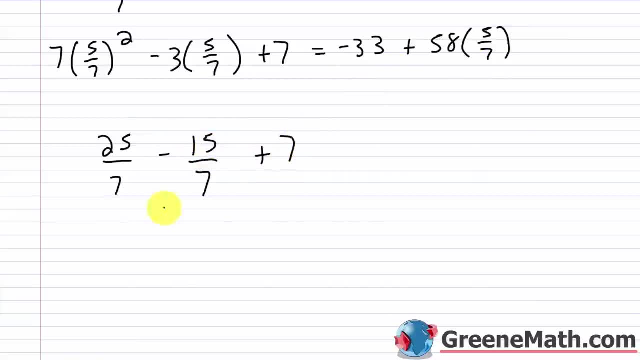 And then plus 7.. Before I go on over here, let me just get a common denominator going, So I could write this as 49 over 7. And then I could just perform the operation with the numerators. 5 minus 15 is 10.. 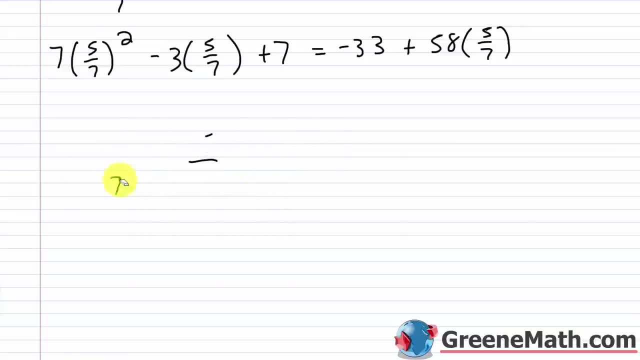 10 plus 49 is 59.. So this is 59 over 7 on the left side. So 59 sevenths, And this equals Over here if I do the multiplication of 58 times 5 sevenths. Well, 58 times 5 is 290.. 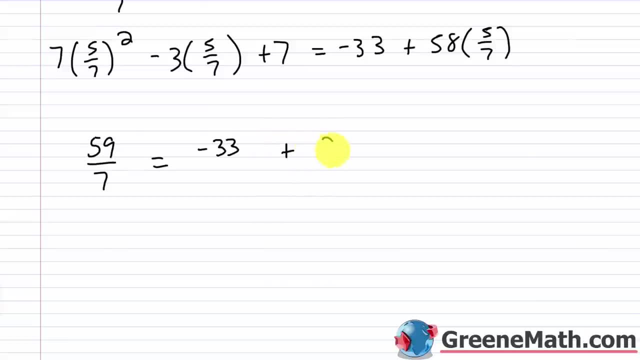 So I'd have negative 33 plus 290 over 7.. Now to get a common denominator here, I'd multiply this by 7 over 7. And I'd get negative 231.. So this would be Negative 231 over 7.. 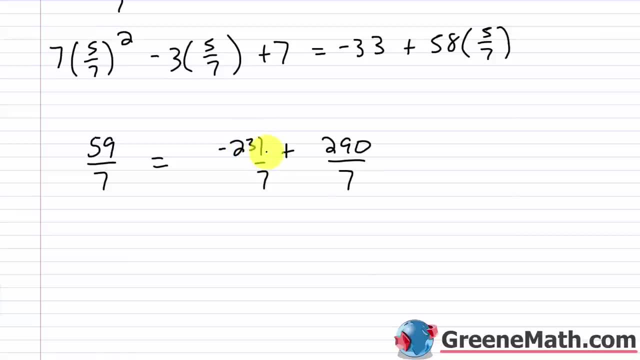 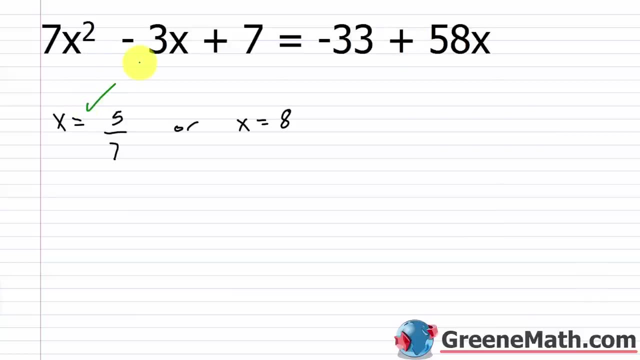 If I do negative 231 plus 290, I get 59. So you'd end up with 59. sevenths is equal to 59 sevenths. So this one checks out. And then the second one is that x equals 8.. 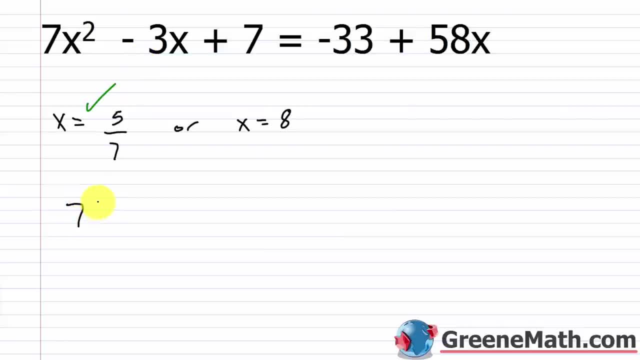 That one's a lot easier to do, So let's knock that out real quick. So, 7 times, You'll have 8 squared minus 3 times 8 plus 7.. This is equal to negative 33 plus 58 times 8.. 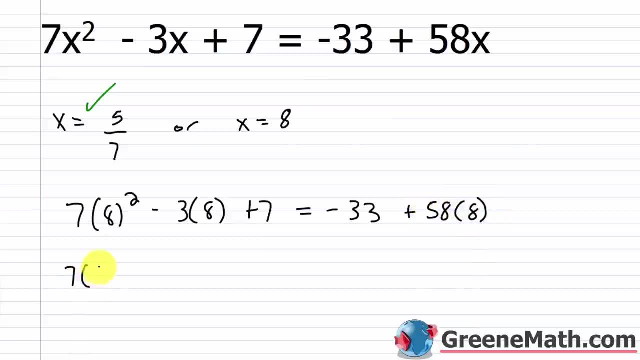 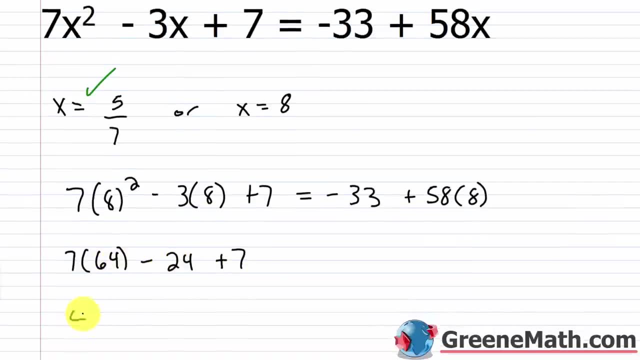 So 8 squared is what, That's 64.. So 7 times 64 minus 3 times 8 is 24 plus 7.. So 7 times 64 is 448.. So 448 minus 24 plus 7.. 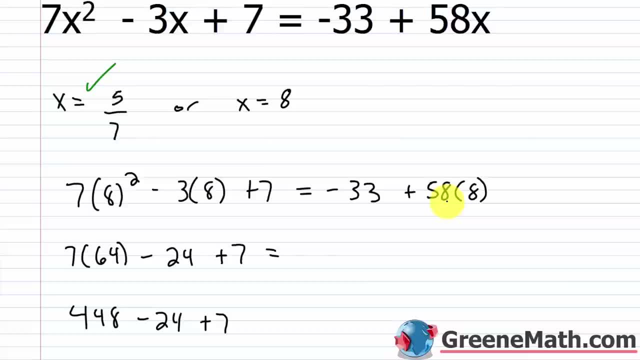 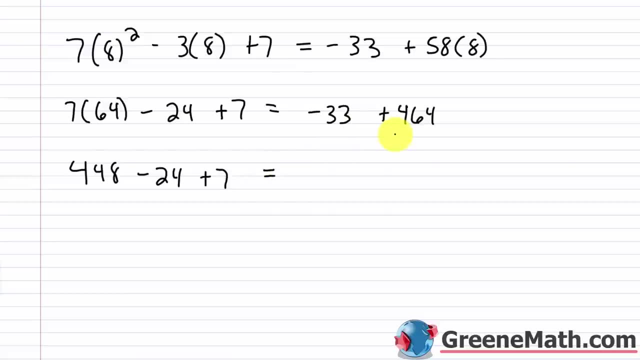 Over here. let's just do some of this: 58 times 8 is 464.. So you'd have negative 33 and then plus 464.. All right, So let's put equals: Negative 33 plus 464 is 431.. 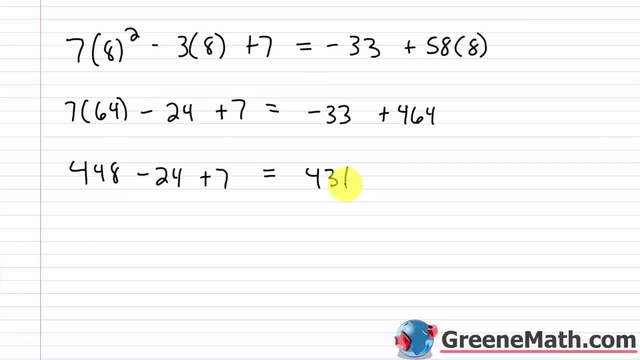 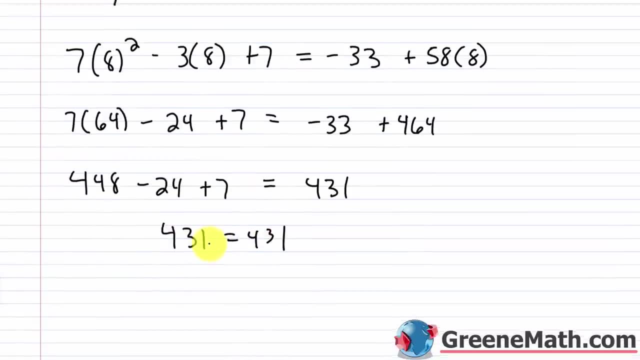 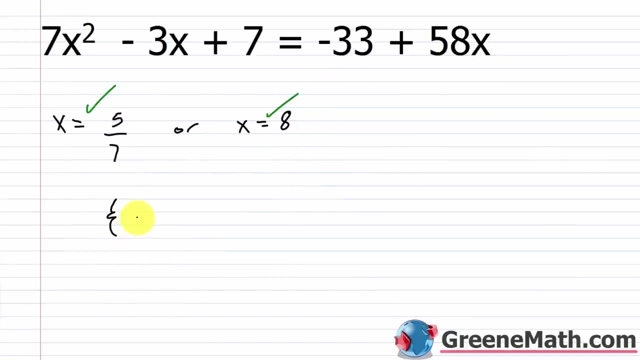 Then over here, 448 minus 24 is 424.. Then plus 7 is 431.. So you get 431 equals 431.. So that works out. So we could say that x equals 8 is also a solution. here And again you can write this in solution set notation: 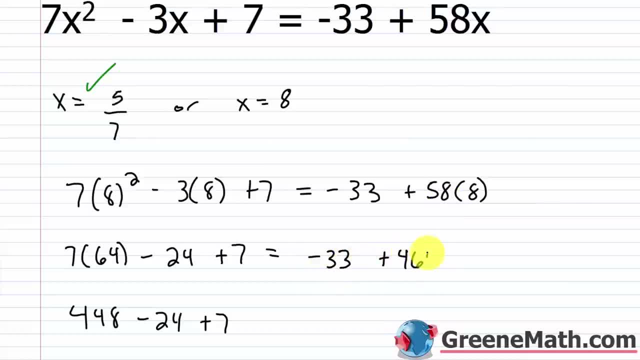 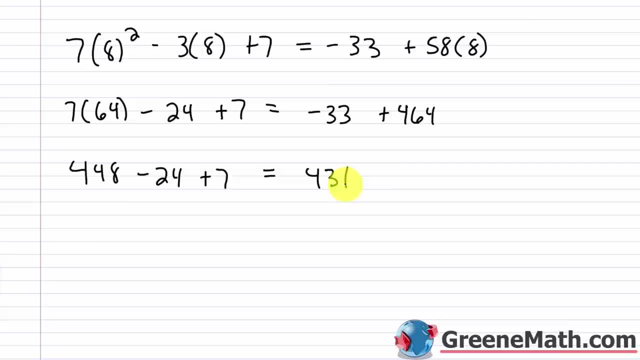 So you'd have negative 33 and then plus 464. All right. So let's put equals negative 33 plus 464 is 431. Then over here, 448 minus 24 is 424. Then plus 7 is 431. So you get 431 equals 431. 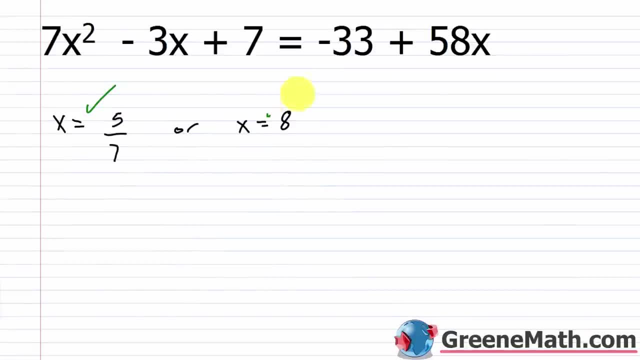 So that works out. So we could say that x equals 8 is also a solution here. And again, you can write this in solution set notation where you'd put 5 7ths comma 8, right? Your two 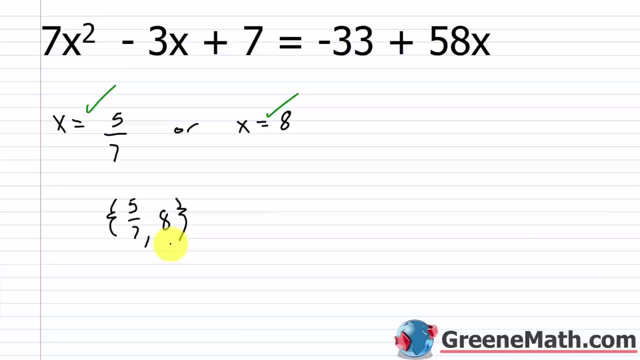 solutions inside of the set braces. But again, in Algebra 1, this is a perfectly acceptable 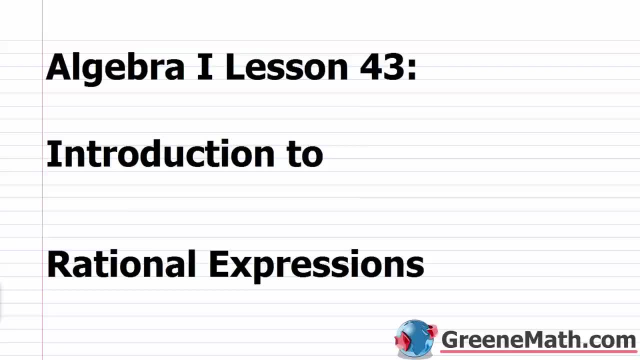 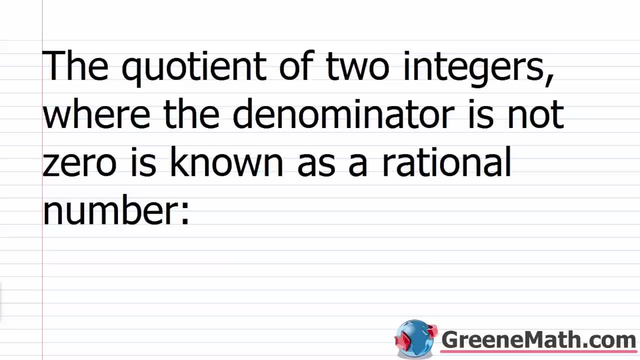 answer. Hello and welcome to Algebra 1, Lesson 43. In this video, we're going to have an introduction to rational expressions. All right. So back in pre-algebra, we learned the definition 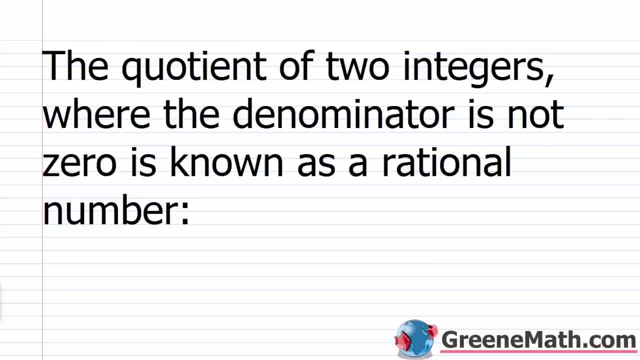 for a whole number and also for an integer. We never really talked about an official definition for a rational number. So the quotient of two integers where the denominator is not zero, because remember, we can never divide by zero, is known as the quotient of two integers. So the quotient of two integers is known as the quotient of two integers. So the quotient of two integers is 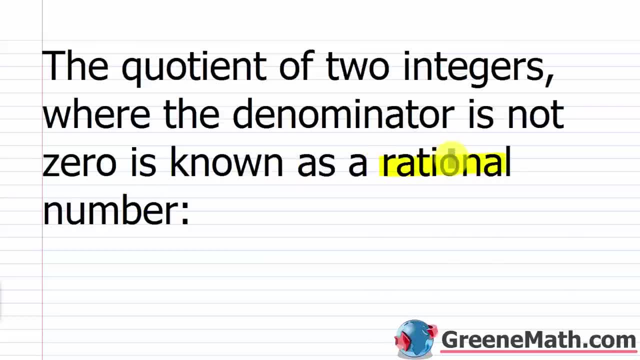 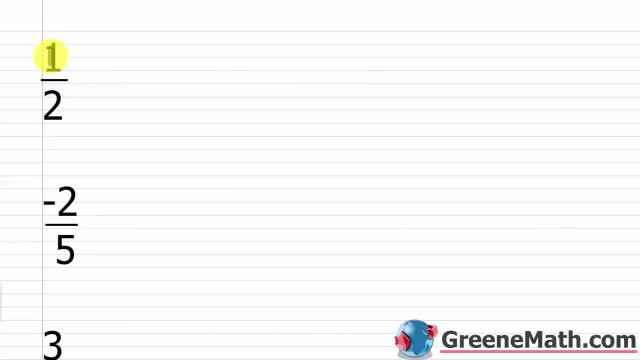 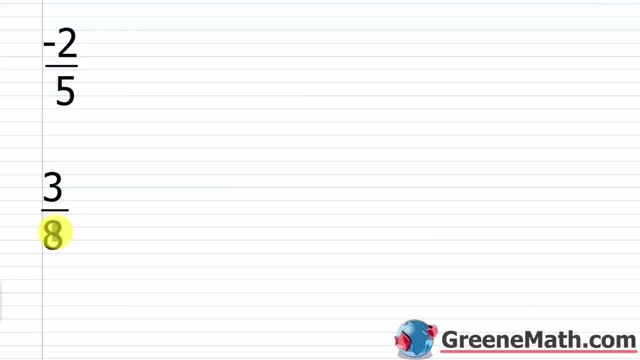 known as a rational number. So this is a rational number. So some examples, you have one half. So this is a rational number. We have an integer of 1 over an integer of 2. Or something like negative two-fifths. You have an integer of negative 2 over an integer of 5. Or as a last example, something like three-eighths. An integer of 3 over an integer of 8. And just so you know, 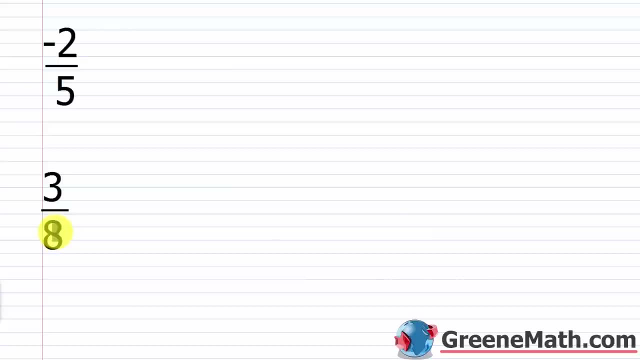 every integer and every whole number can be written as a rational number by just simply writing the number over 1. If I had the number, let's say, 3, I could just write 3 over 1, and now it's a rational number. Or if I had something like negative 7, I could write negative 7 over 1, and now it's a rational number. Where you would run into a problem, 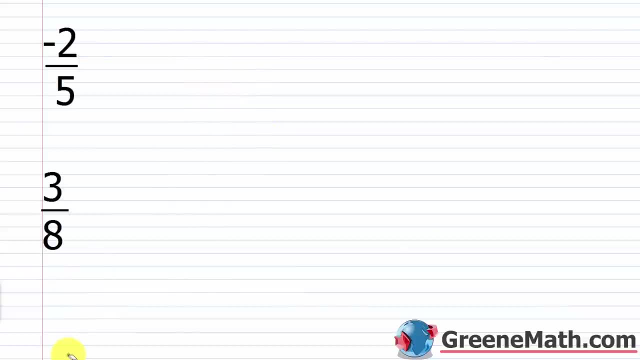 and you're going to see this later on, if you have something like, let's say, the square root of 5. So the square root of 5. I cannot write this number as the, the quotient of two integers, no matter how hard I try. I can't just say, 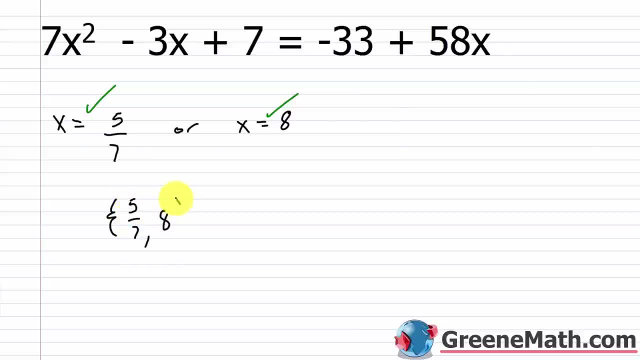 where you'd put 5, sevenths comma 8.. Right, Your two solutions inside of the set braces, But again in Algebra 1, this is a perfectly acceptable answer. Hello And welcome to Algebra 1,, Lesson 43.. 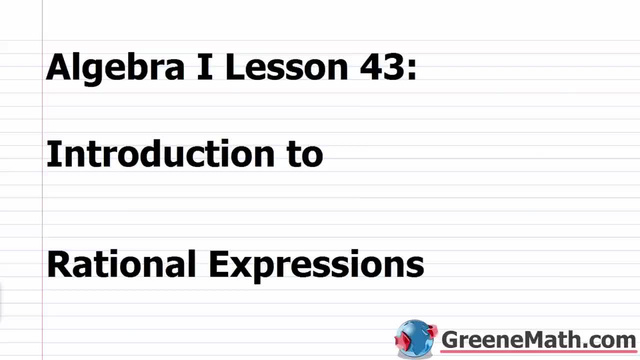 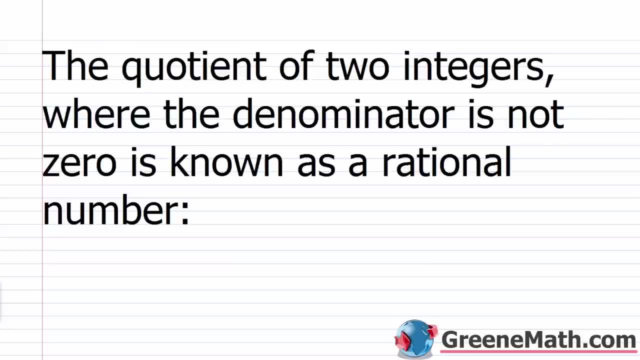 In this video we're going to have an introduction to rational expressions. All right. So back in pre-algebra we learned the definition for a whole number and also for an integer. We never really talked about an official definition for a rational number. 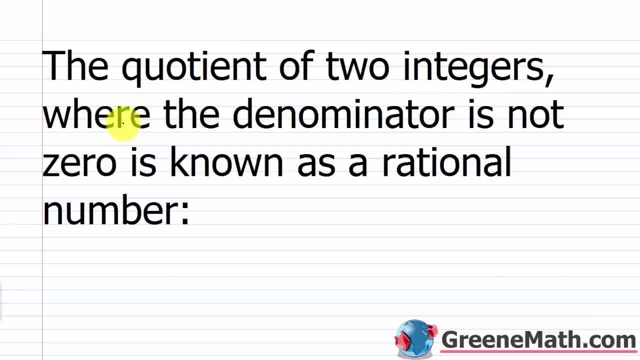 So the quotient of two integers where the denominator is not 0,- because, remember, we can never divide by 0, is known as a rational number. OK, So this is a rational number. So some examples you have: 1 half. 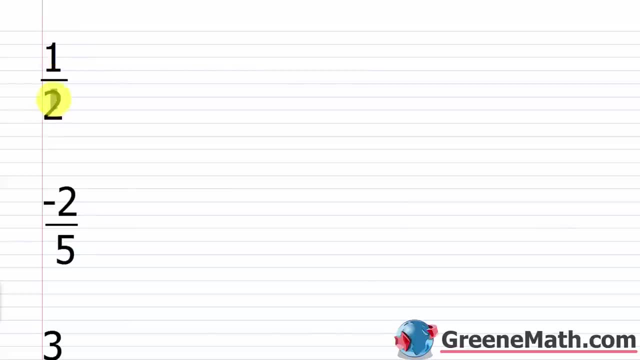 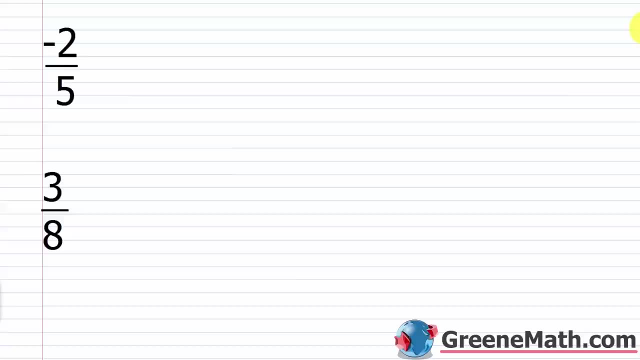 So this is a rational number. We have an integer of 1 over an integer of 2.. Or something like negative 2: fifths, You have an integer of negative 2 over an integer of 5.. Or, as a last example, something like 3: eighths. 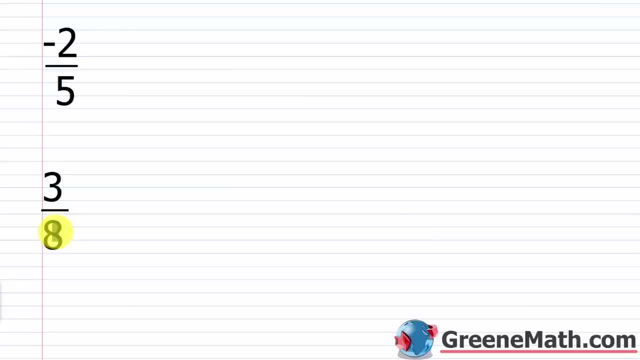 An integer of 3 over an integer of 8.. And just so you know, every integer and every whole number can be written as a rational number by just simply writing the number over 1.. All right, If I had the number, let's say 3, I could just write 3 over 1.. 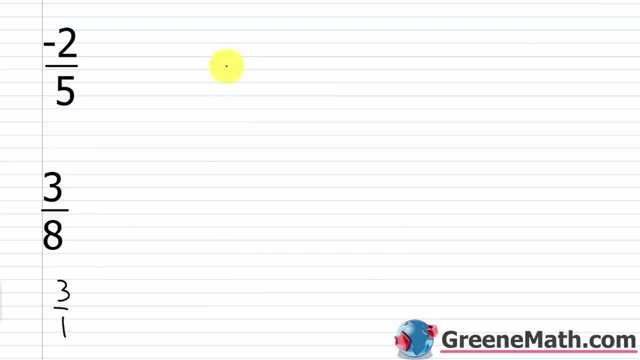 And now it's a rational number. Or if I had something like negative 7, I could write negative 7 over 1.. And now it's a rational number Where you would run into a problem, and you're going to see this later on. 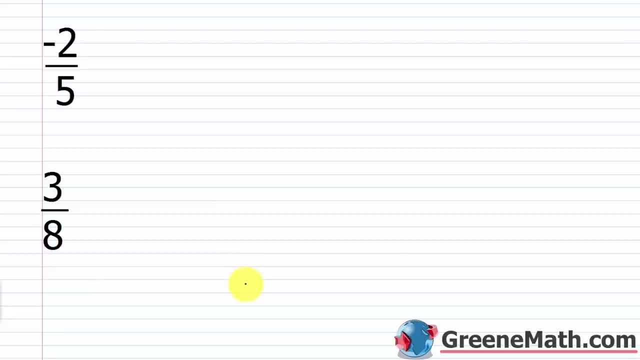 if you have something like, let's say, the square root of 5.. So the square root of 5.. I cannot write this number as the quotient of two integers, no matter how hard I try. I can't just say, OK, square root of 5 over 1.. 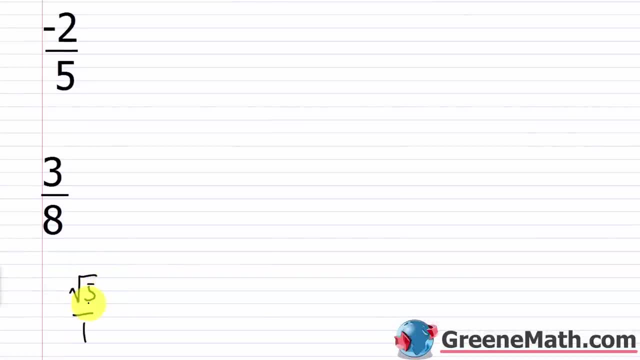 That's not going to work because this part right here, the numerator, is not an integer, So this is known as an irrational number, And we're going to study those a little bit later on in Algebra 1.. All right, so kind of moving forward here. 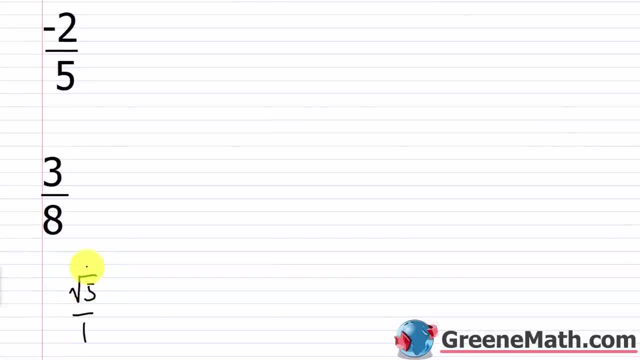 okay, square root of 5 over 1. That's not going to work, because this part right here, the numerator, is not an integer. So this is known as an irrational number, and we're going to study 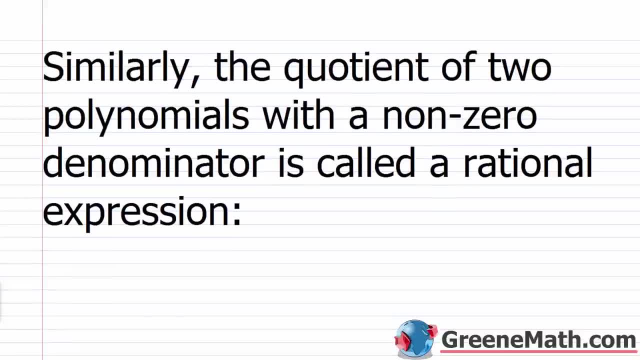 those a little bit later on in Algebra 1. All right, so kind of moving forward here, I want to just say that similarly, the quotient of two polynomials, okay, the quotient of two polynomials, with again, a non-zero denominator, because you can't divide by zero, is called a rational expression. This is what we're going to learn about today, 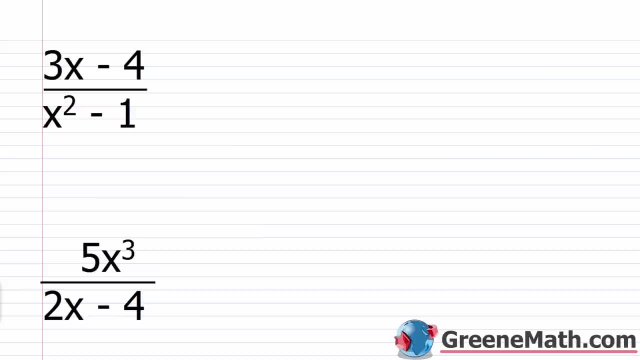 a rational expression. So here are some examples. You have 3x minus 4 over x squared minus 1. So you have a polynomial in your numerator, a polynomial in your denominator. So then this 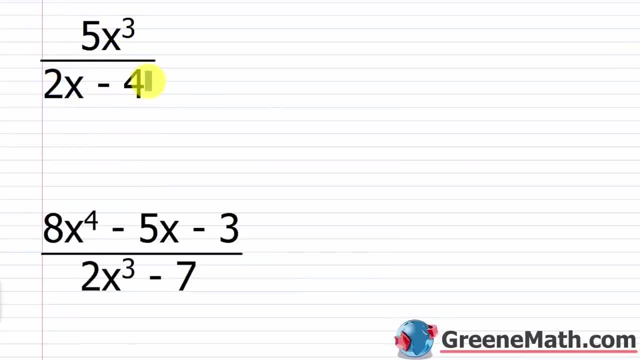 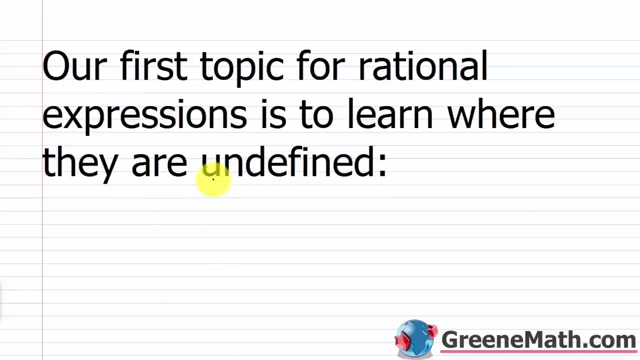 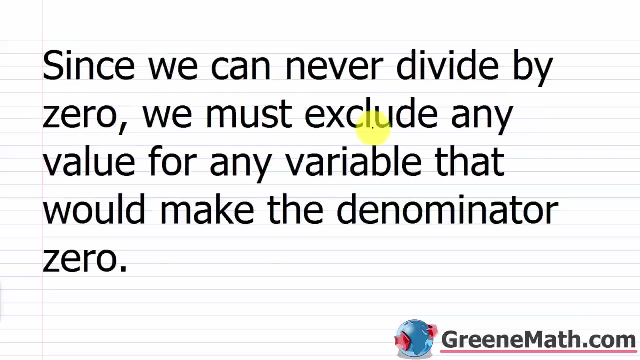 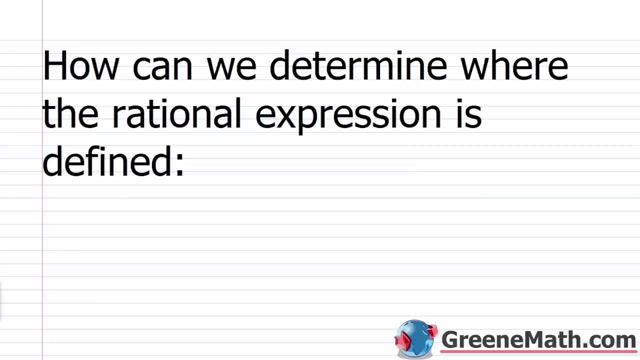 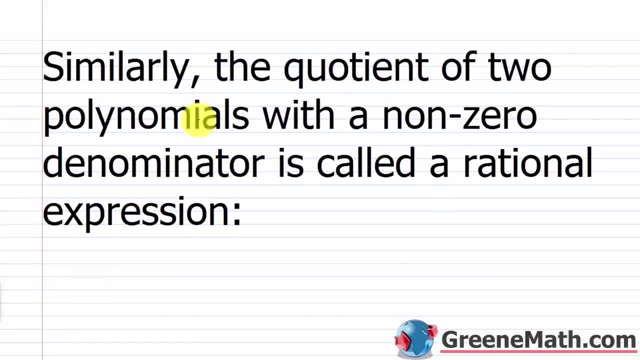 I want to just say that, similarly, the quotient of two polynomials- the quotient of two polynomials with, again, a non-zero denominator, because you can't divide by 0, is called a rational expression, And this is what we're going to learn about today: a rational expression. 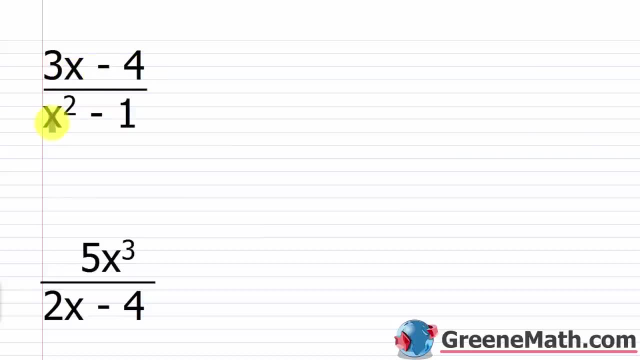 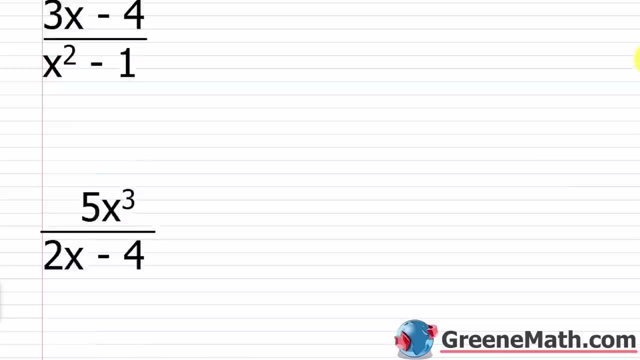 So here are some examples: You have 3x minus 4 over x squared minus 1.. So you have a polynomial in your numerator, a polynomial in your denominator. So then this one: right here you have 5x cubed over 2x minus 4.. 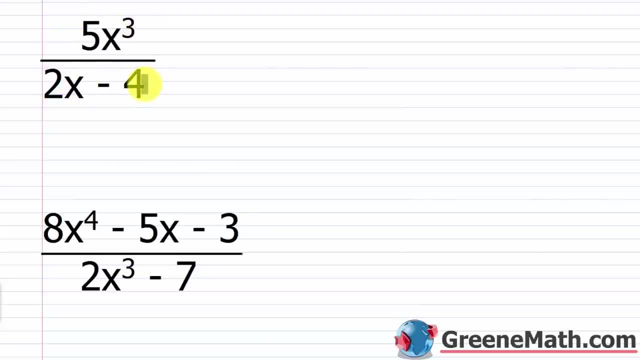 So you have a polynomial in the numerator over a polynomial in the denominator. And then here you have 8x to the fourth power minus 5x, minus 3 over 2x cubed minus 7.. I got a polynomial in the numerator over a polynomial in the denominator. 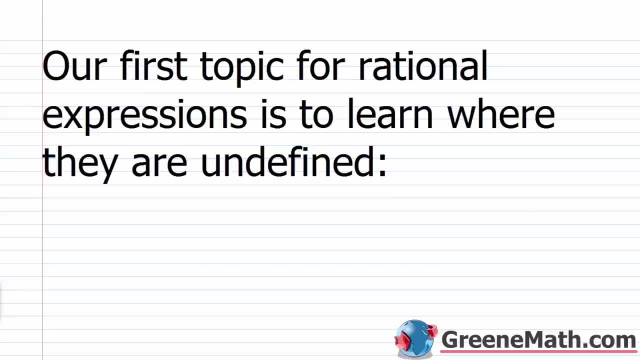 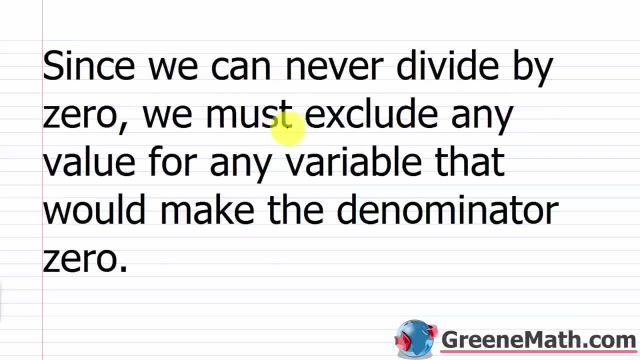 So our first topic for rational expressions is simply to learn where they are undefined, And this has to do with division by 0.. So since we can never divide by 0, we must exclude any value for any variable that would make the denominator 0. 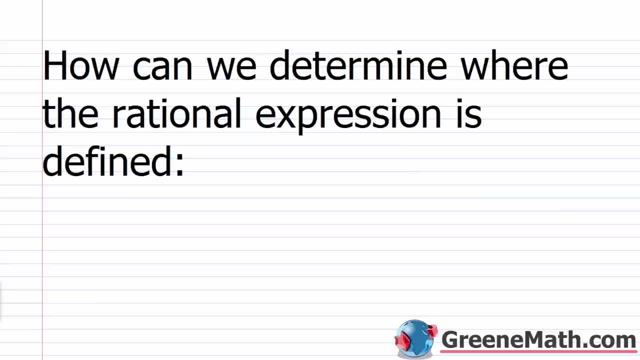 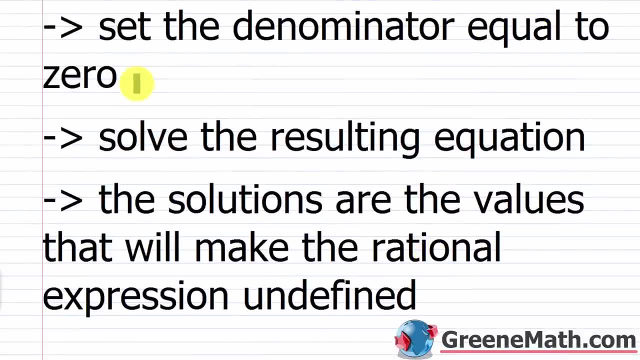 Very, very important. So how can we determine where the rational expression is defined? Well, it's actually kind of easy. We already have all the skills to do it. We just want to set the denominator equal to 0. We want to solve the resulting equation. 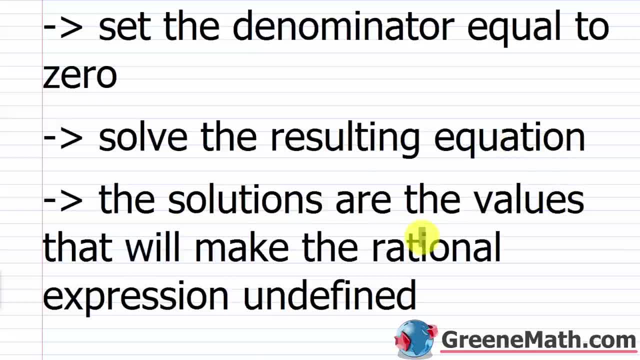 And then the solutions are the values that will make the rational expression undefined, Because if we set it equal to 0 and we solve for those values, those values would make the denominator 0, and that's not allowed. So here's an example. 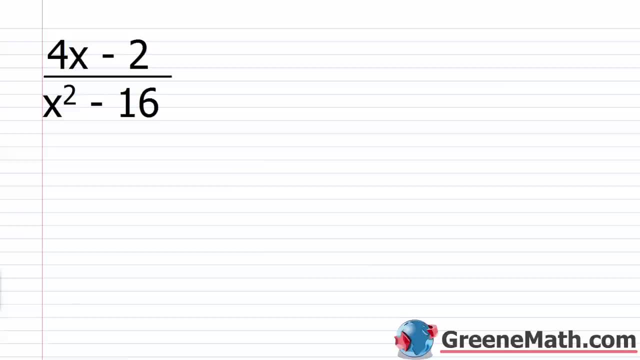 We have 4x minus 2 over x squared minus 16.. So we know that this cannot be 0. Cannot be 0. So how do we figure out what values would make it 0? We just set it equal to 0.. 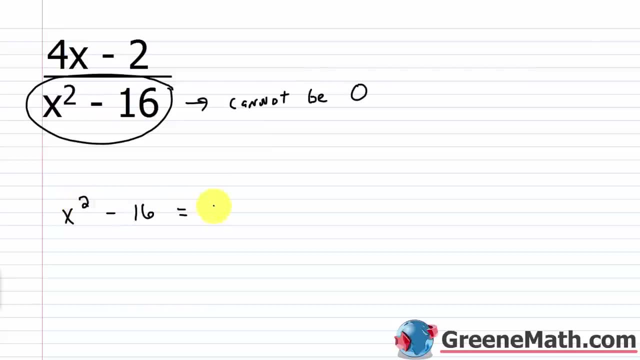 So we say x squared minus 16 is equal to 0.. In the last lesson we learned how to solve a quadratic equation by factoring. Now, if you get something in your denominator that you can't factor, if you get a quadratic equation, you can't factor. 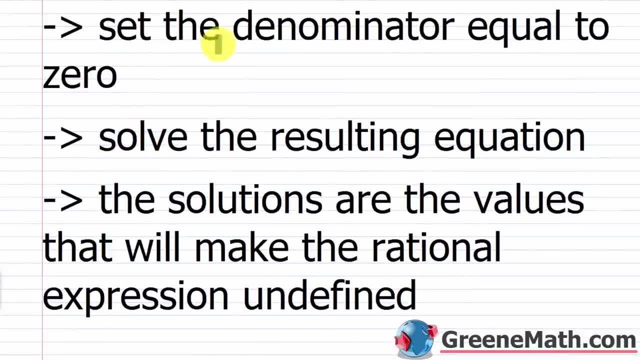 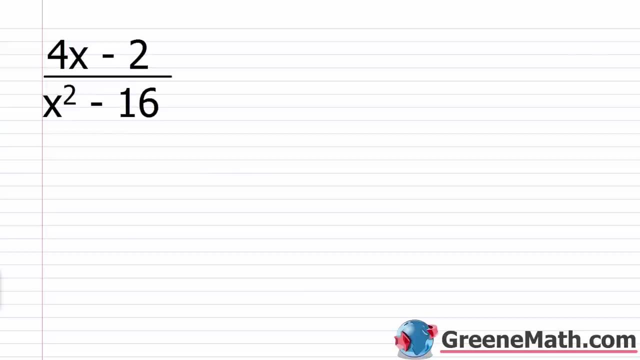 Well, it's actually kind of easy. We already have all the skills to do it. We just want to set the denominator equal to zero. We want to solve the resulting equation. And then the solutions are the values that will make the rational expression undefined. Because if we set it equal to zero and we solve for those values, those values would make the denominator zero, and that's not allowed. So here's an example. We have 4x minus 2 over x squared minus 16. So we know that this cannot be zero. Cannot be zero. So how do we figure out what values would make it zero? We just set it equal to zero. So we say x squared minus 16 is equal to zero. In the last lesson, we learned how to solve a quadratic equation by factoring. Now, if you get something in your denominator that you can't factor, if you get a quadratic equation you can't factor, you're not going to be able to deal with that until we get to the denominator. 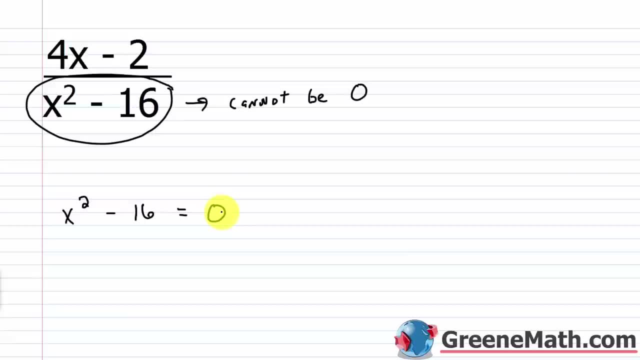 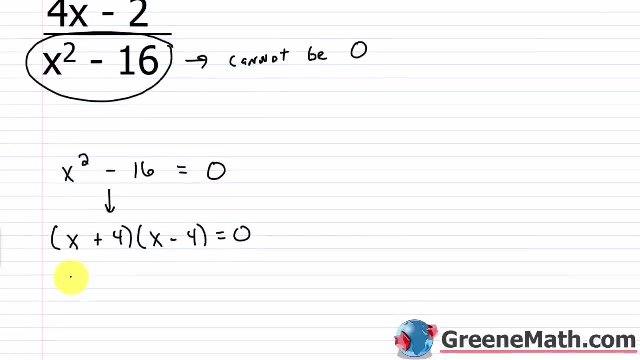 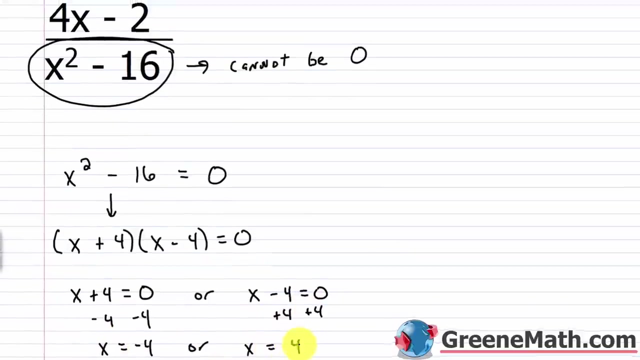 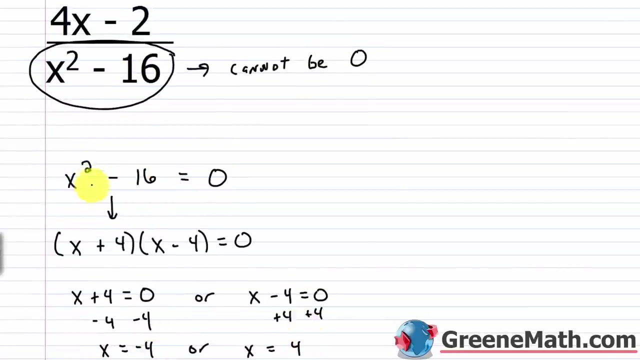 So we get to completing the square and solving quadratic equations using the quadratic formula. And that's all the way at the end of Algebra 1. So right now I'm just going to give you stuff you can factor so you just get used to this. So we have x squared minus 16 equals zero. We know this is the difference of two squares. So I can factor this as x plus 4 times x minus 4 equals zero. And we know from our zero product property that x plus four and then we put or x minus 4 is set equal to 0. If we solve these two equations, subtract 4 away from here and here, I get x equals negative 4, or add 4 to both sides of the equation, I get x is equal to 4. And if you check these, negative 4 squared is 16, 16 minus 16 is 0, and then 4 squared is 16, 16 minus 16 is 0, so they both work out. So what we would say is that replacing the variable x here with a 4 or a negative 4 would result in a value of 0 for the denominator, and that's not allowed. So your restricted values here 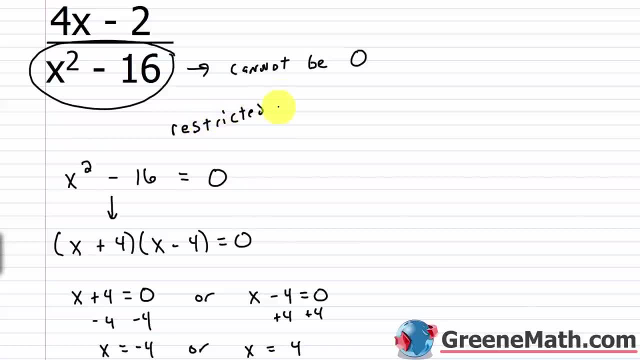 for x are 4 and negative 4, right? x cannot be equal to 4 or negative 4. 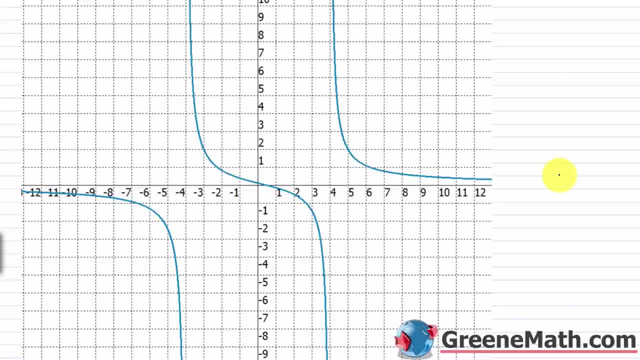 So before we kind of move on, I just want to show you what this looks like graphically. Again, I'm going to show you how I do the multiple numbers here. So I'm just going to 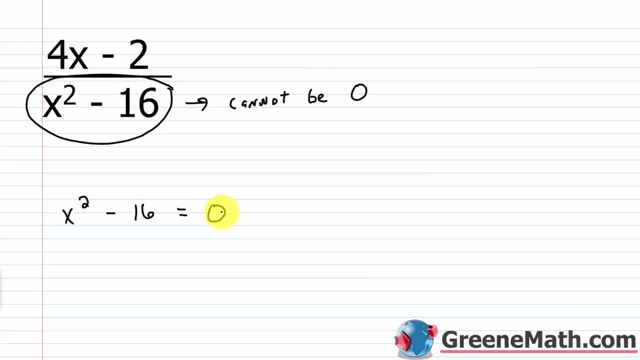 you're not going to be able to deal with that until we get to completing the square and solving quadratic equations using the quadratic formula, And that's all the way at the end of Algebra 1.. So right now I'm just going to give you stuff you can factor, so you just get used to this. 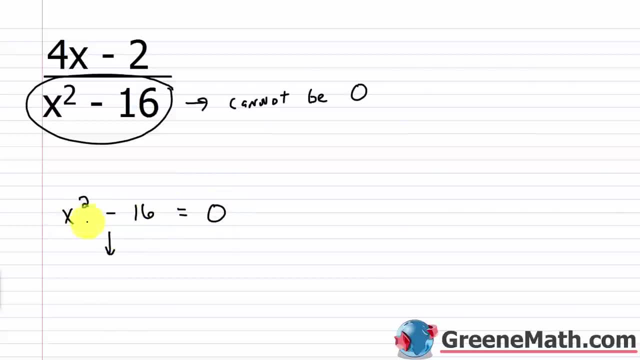 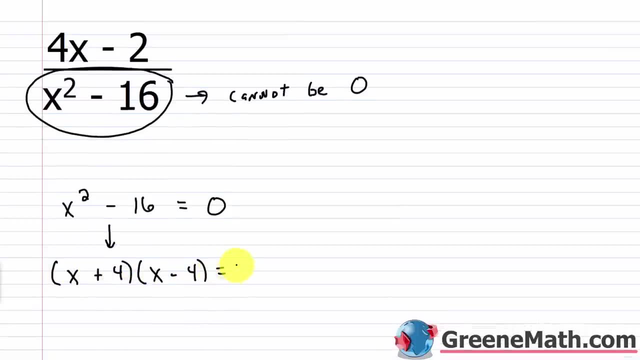 So we have x squared minus 16 equal to 0.. We know this is the difference of two squares, so I can factor this as x plus 4 times x minus 4, equal to 0.. And we know from our zero product property that x plus 4 is set equal to 0.. 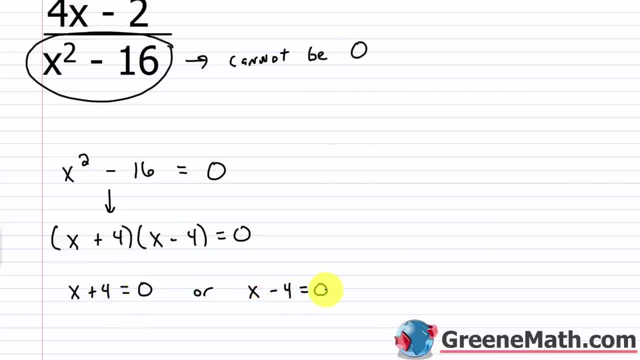 And then we put: or x minus 4 is set equal to 0.. If we solve these two equations, subtract 4 away from here and here, I get x equals negative 4, or add 4 to both sides of the equation, I get x is equal to 4.. 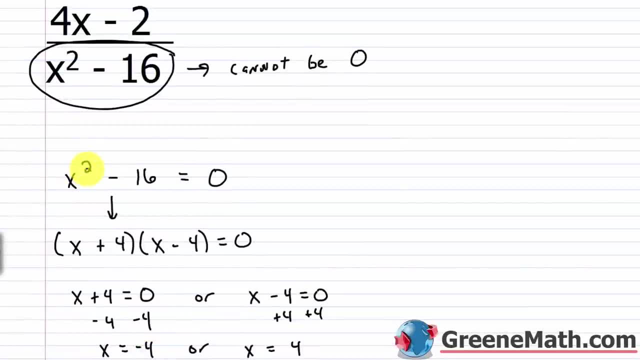 And if you check these negative, 4 squared is 16, 16 minus 16 is 0, and then 4 squared is 16, 16 minus 16 is 0, so they both work out. So what we would say is that, replacing the variable x, 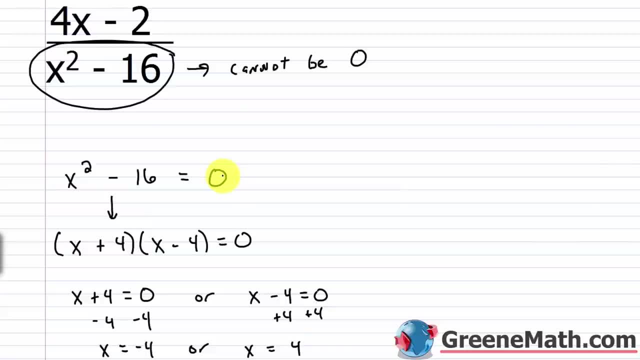 here with a 4 or a negative 4 would result in a value of 0 for the denominator, and that's not allowed. So your restricted values here for x are 4 and negative 4, right x cannot be equal to 4. 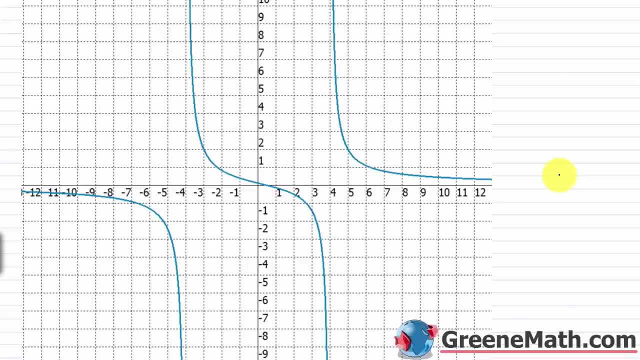 or negative 4.. So, before we kind of move on, I just want to show you what this looks like graphically. If you were to graphically graph 4x minus 2 over x squared minus 16,, what you would get is a graph that looks like this: 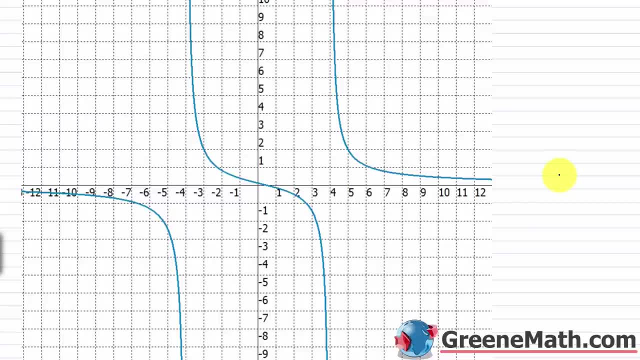 And depending on what you set your maximum range to be, it might be a little bit different. Some computers draw it a little differently. but the main thing to notice here is that look at when x is 4 and when x is negative 4.. Remember we said x couldn't be 4 or negative 4.. Look at the fact. 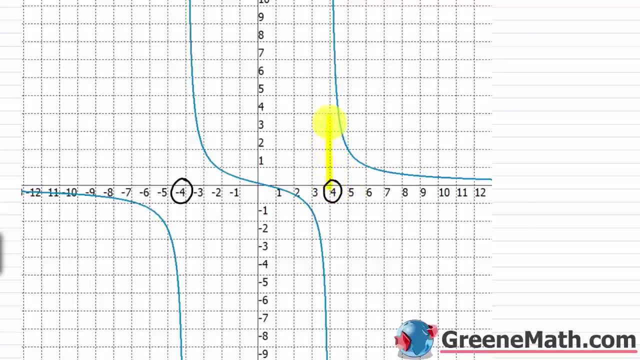 that on your y-axis, the graph is never going to actually touch that point. I'm trying to make this as straight as I can. It gets very, very, very close to that, but it never touches it. And the same thing going down. 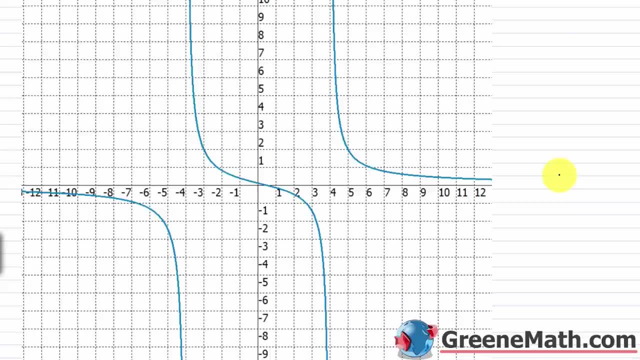 If you were to graph 4x minus 2 over x squared minus 16, what you would get is a graph that looks like this. 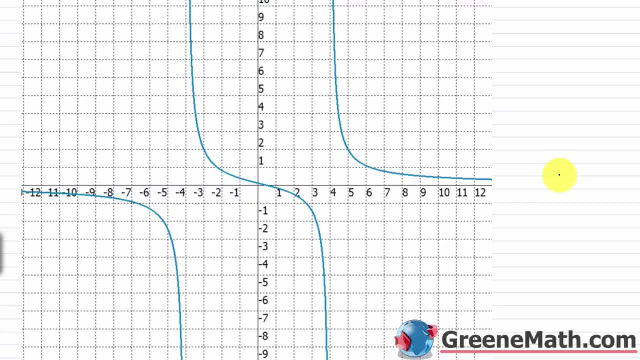 And depending on what you set your maximum range to be, it might be a little bit different. Some computers draw it a little differently. But the main thing to notice here is that look at when x is 4 and when x is negative 4. 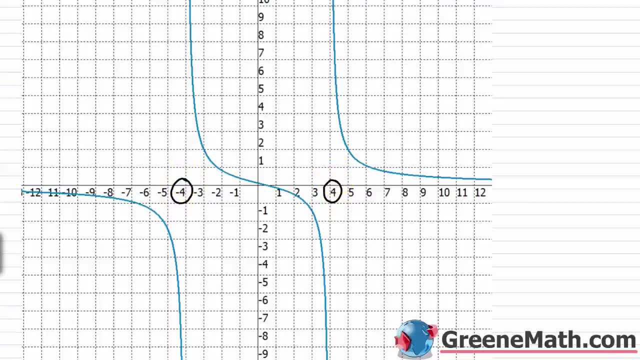 Remember, we said x couldn't be 4 or negative 4. Look at the fact that on your y-axis, the graph is never going to actually touch that point. I'm trying to make this as straight as I can. It gets very, very, very close to that, but it never touches it. And the same thing going down here. It gets very, very, very close to that, but it's never gonna touch it. 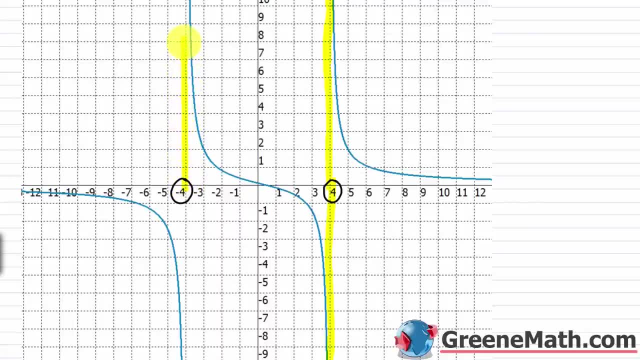 And then same thing over here. It gets very, very close to it, but it's never gonna touch it. Very, very close, never gonna touch it. And these things are called asymptotes. 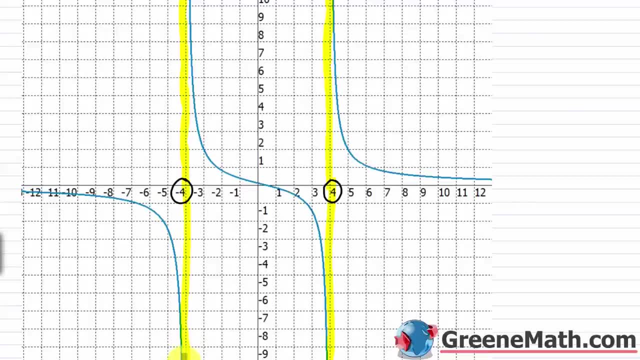 And we're gonna talk about these a lot in Algebra 2 when we start graphing really heavily. 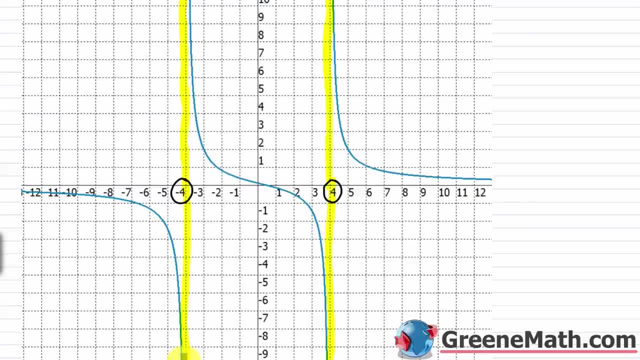 But for right now, I just wanna give you a little insight into what this looks like. 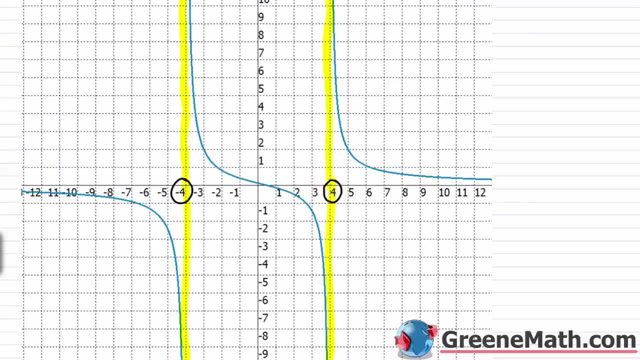 So when x is 4, there's no value for y that's corresponding to that. And then also when x is negative 4, there's no value for y that's corresponding to that on that graph, right? 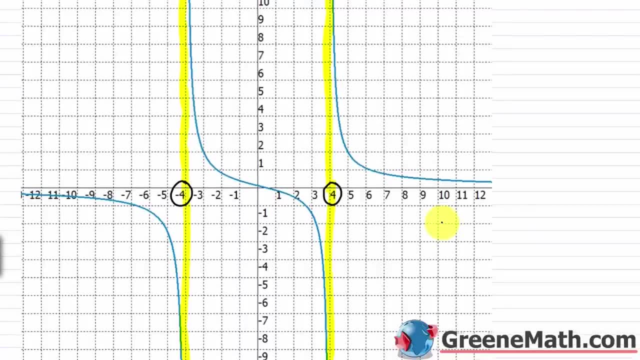 Again, that's because x is not allowed to be 4 or negative 4. 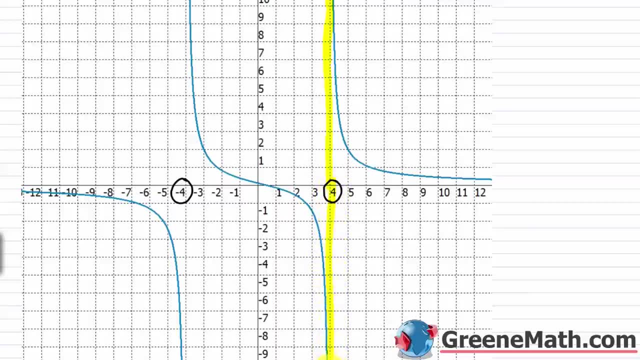 here, It gets very, very, very close to that, but it's never going to touch it. And then same thing over here: It gets very, very close to it, but it's never going to touch it- Very, very close. 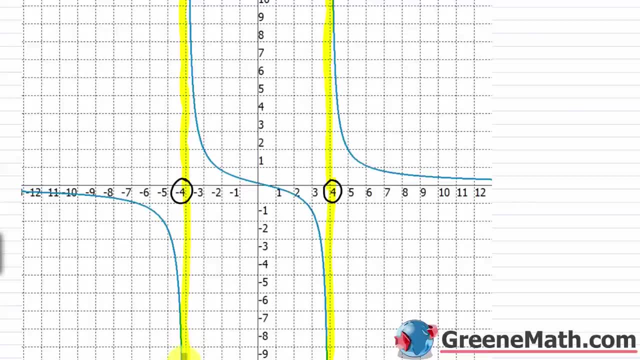 never going to touch it, And these things are called asymptotes, And we're going to talk about these a lot in Algebra 2 when we start graphing really heavily, But for right now I just want to give you a little insight into what this looks like. So 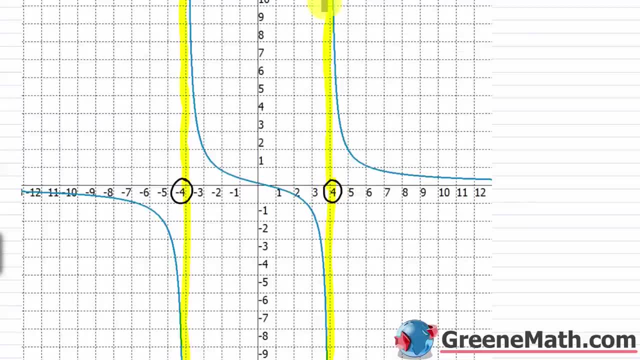 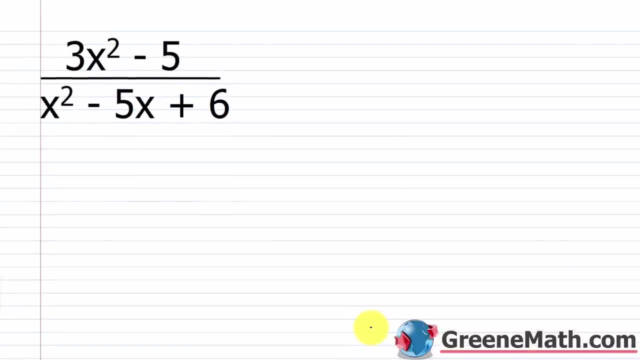 when x is 4, there's no value for y. that's corresponding to that. And then also when x is negative 4, there's no value for y- that's corresponding to that on that graph. Again, that's because x is not allowed to be 4 or negative 4.. Let's take a look at another one. 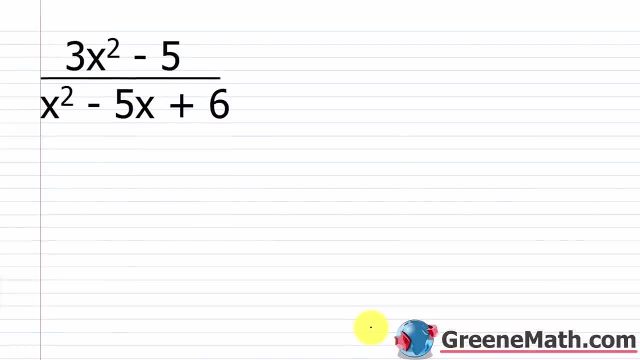 So we have 3x squared minus 5 over x squared minus 5x plus 6.. So again, the denominator cannot be 0.. to make it zero is to plug in values for x that result in this becoming zero. So what I would do, 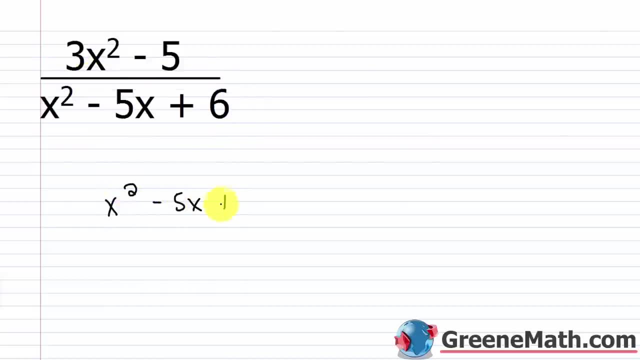 is, I would say: okay, x squared minus 5x plus 6, set it equal to zero, find out what those values are, and then those are going to be the values that are restricted. So this is a factorable trinomial. So I can factor this into the product of two binomials And this is pretty easy Give. 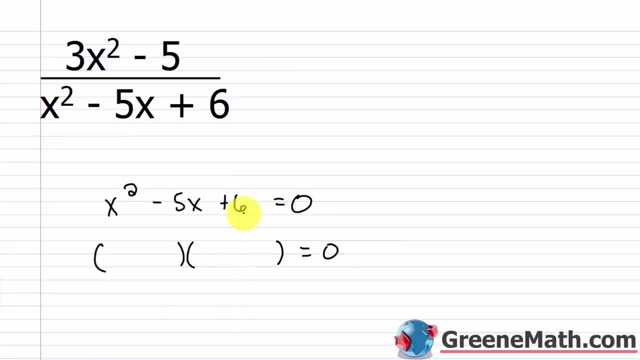 me two integers whose sum is negative 5, whose product is 6. So that would be negative 2 and negative 3.. Negative 2 times negative 3 is 6.. Negative 2 plus negative 3 is negative 5.. 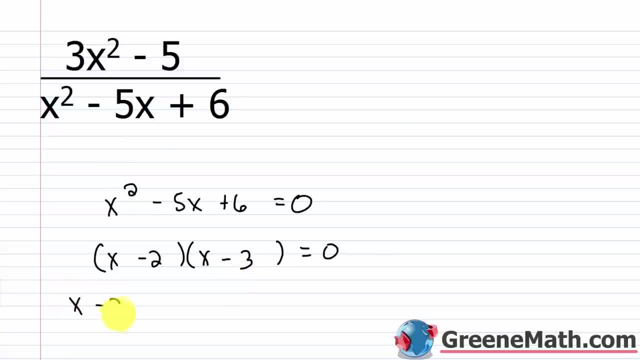 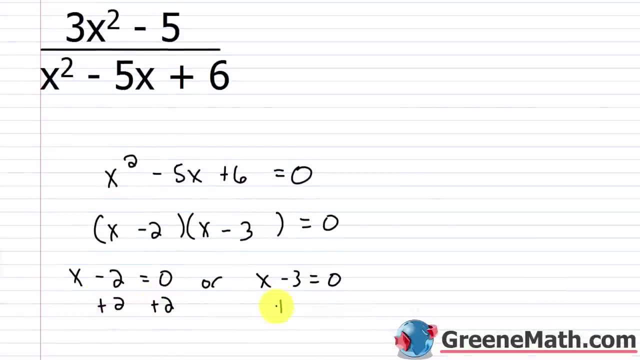 So then I would set each of these equal to zero and I would solve individually. So if I add 2 to both sides over here, if I add 3 to both sides over here, I'd get x equals 2 or x equals 3.. 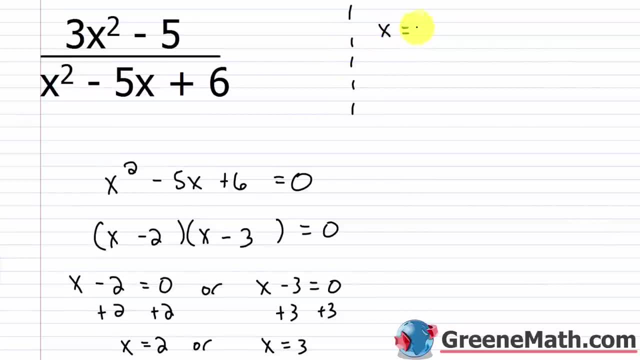 So I'll put over here: x equals 2 or x equals 3.. You can check those real quick. Plug in a 2 here and here You would get 2 squared, that's 4.. And then, so this is 4, and then minus 5 times 2 is. 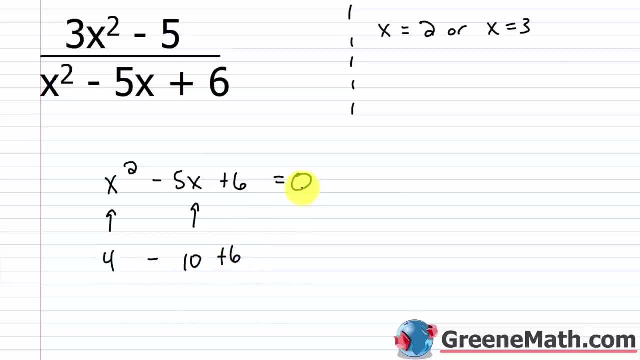 10 plus 6.. 4 plus 6 is 10.. 10 minus 10 is zero. So that one checks out And then I can replace these: Put 3 squared here, that's 9.. Negative 5 times 3, that's negative 15.. So 9 plus 6 is 15.. Okay, let's take a look at another one. So we have 3x squared minus 5 over x squared minus 5x, plus 6. 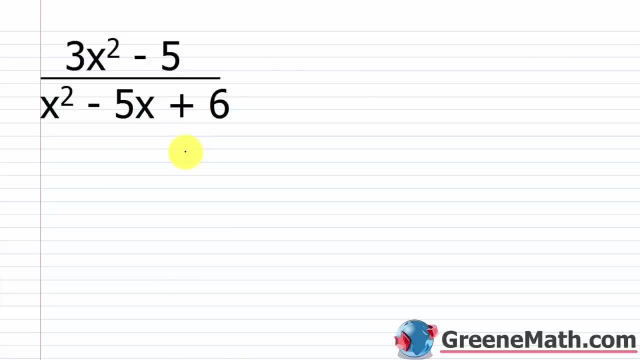 So again, the denominator cannot be 0. The only way to make it 0 is to plug in values for x 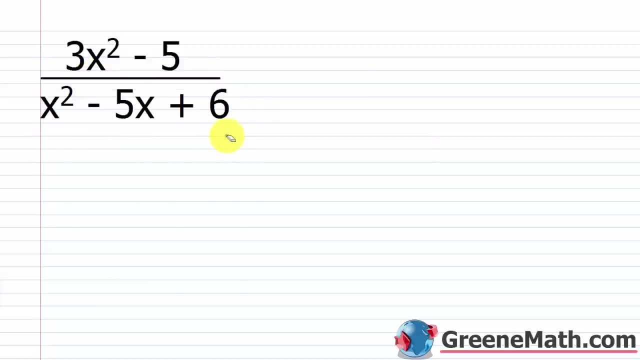 that result in this becoming 0. So what I would do is I would say, okay, x squared minus 5x plus 6, set it equal to 0, find out what those values are, and then those are gonna be the values that are restricted. 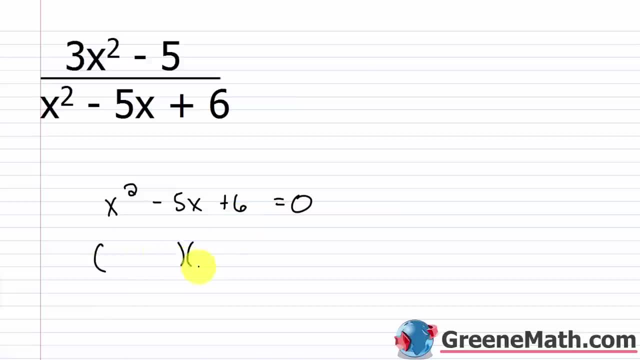 So this is a factorable trinomial. So I can factor this into the product of two binomials. And this is pretty easy. Give me two integers whose sum is negative 5, whose product is 6. So that would be negative 2 and negative 3. Negative 2 times negative 3 is 6. Negative 2 plus negative 3 is negative 5. So then I would set each of these equal to 0, and I would solve individually. 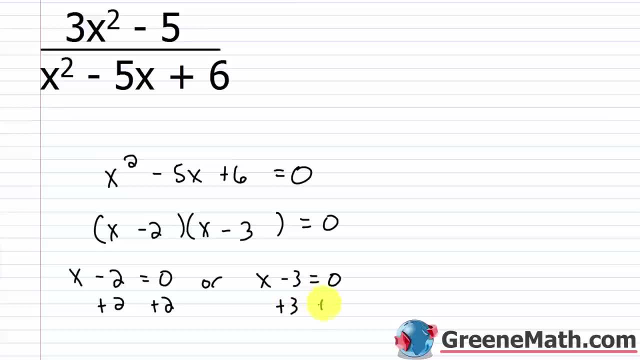 So if I add 2 to both sides over here, and if I add 3 to both sides over here, I'd get x equals 2 or x equals 3. So I'll put over here, 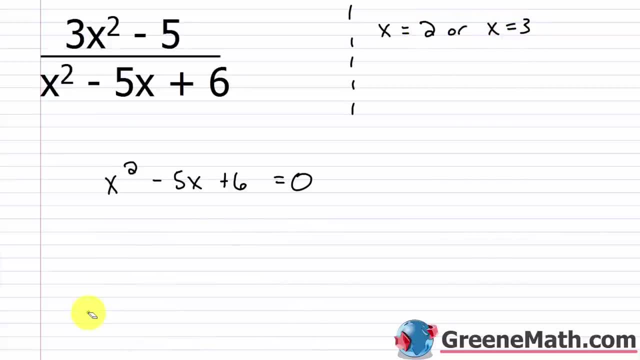 x equals 2 or x equals 3. You can check those real quick. 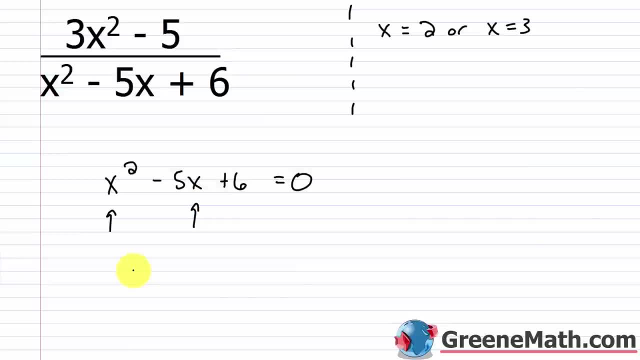 Plug in a 2 here and here. You get 2 squared, that's 4. And then, so this is 4, and then minus 5 times 2 is 10 plus 6. 4 plus 6 is 10, 10 minus 10 is 0. So that one checks out. 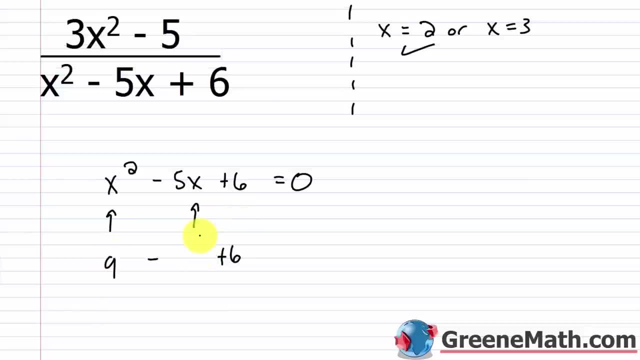 And then I can replace these, put 3 squared here, that's 9. Negative 5 times 3, that's negative 15. So 9 plus 6 is 15. 15 minus 15 is 0. That checks out as well. So our restricted values here are 2 and 3. So x 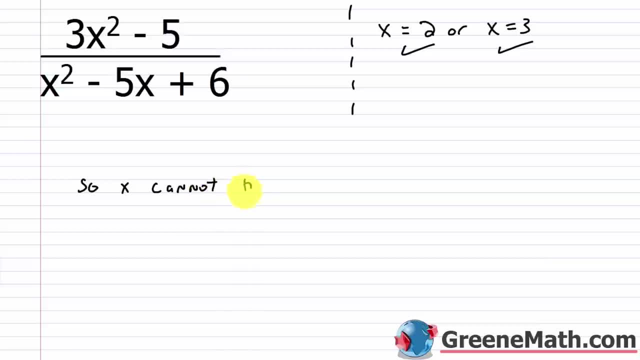 cannot be 2 or 3. And when we get to Algebra 2, I'll give you kind of a fancier way to write that. I just want you to have an understanding of sets before we kind of jump into that. 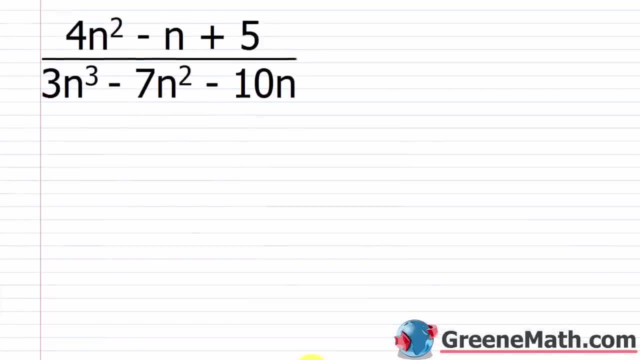 Okay, let's take a look at one more of these. It's pretty simple overall. So we have 4n squared minus n plus 5 over 3n cubed minus 7n squared minus 10n. 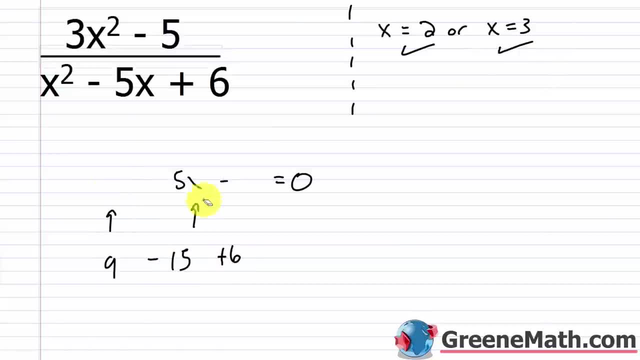 15 minus 15 is 0. That checks out as well. So our restricted values here are 2 and 3.. So x cannot be 2 or 3.. And when we get to algebra 2, I'll give you kind of a fancier way to write that. 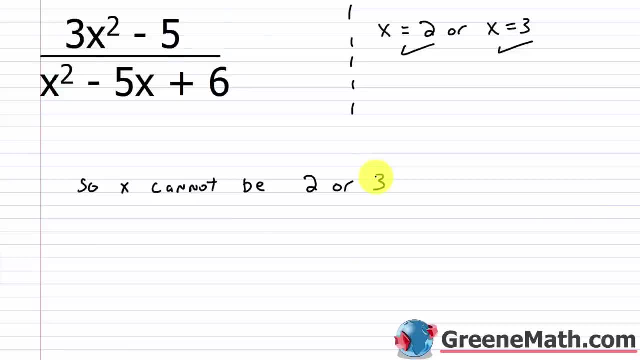 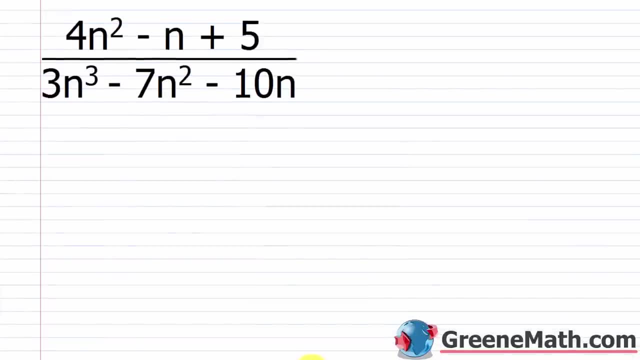 I just want you to have an understanding of sets before we kind of jump into that. Okay, let's take a look at one more of these. It's pretty simple overall. So we have 4n squared minus n plus 5 over 3n cubed minus 7n squared. 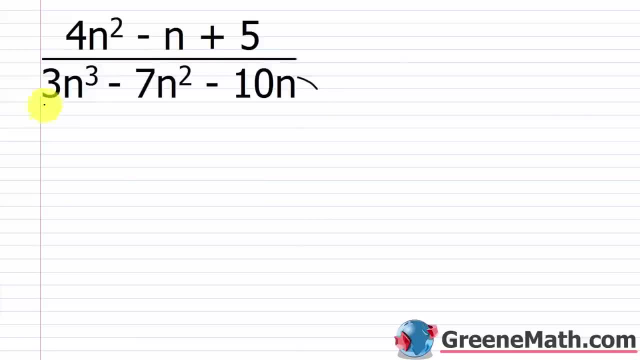 minus 10n. So again, all I want to do is take my denominator, whatever it is, and set it equal to zero and find out what the restricted values are. So 3n cubed minus 7n squared minus 10n. Again, set this equal to zero And I'm going to find out what values of n. 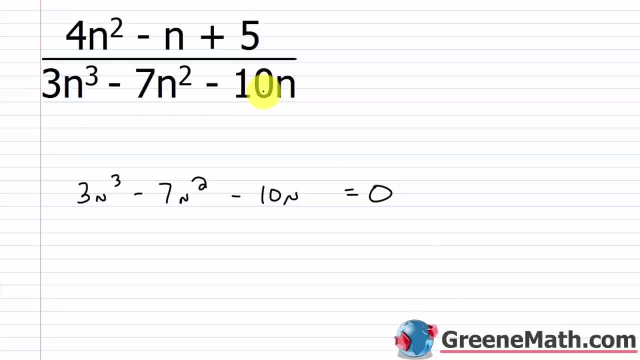 are going to make this denominator zero, And that's again what we can't have. Those are the restricted values. So, to factor this, I notice that I have an n. that's common to everything, So let's pull that out to start. 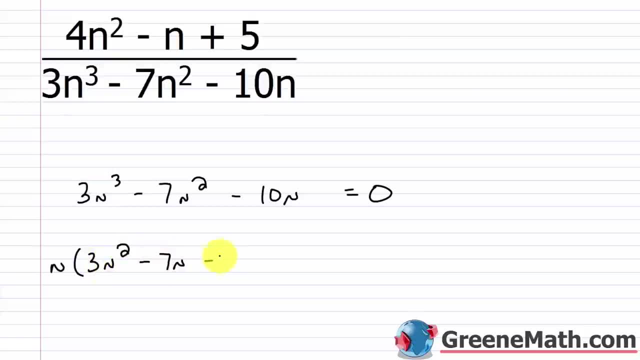 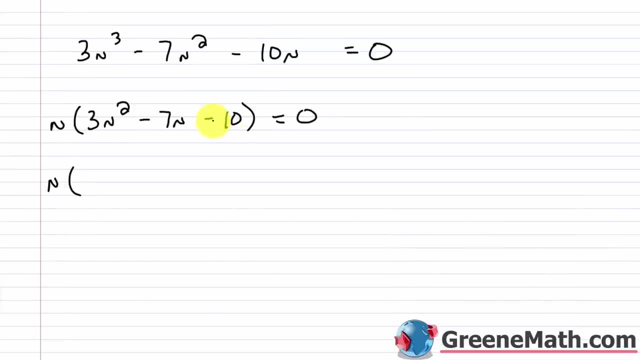 So we'd have 3n squared minus 7n minus 10.. This equals zero. And then to factor this, I'm going to use the grouping method And I want you to give me two integers whose product is negative 30 and whose sum is negative 7.. Well, that's pretty easy If you think about 10 and 3,. 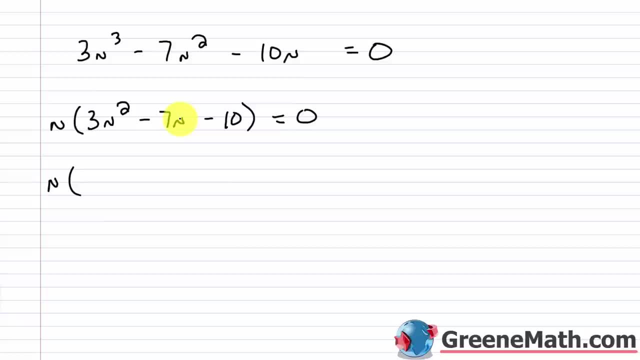 10 times 3 is 30. And I can manipulate the signs to get to negative 7.. So if I think about negative 10 and positive 3, that gives me exactly what I want. So 3n squared, Then I'm going to put plus 3n. 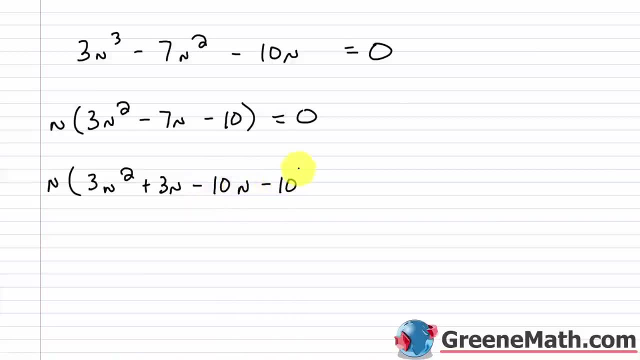 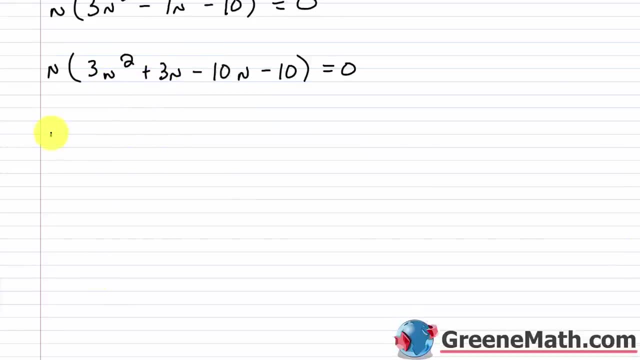 And then minus 10n, And then minus 10.. This equals zero. Again I'm going to be factoring by grouping, So out of this first group I can pull out a 3n. So I'm going to have n times Pull out a 3n. 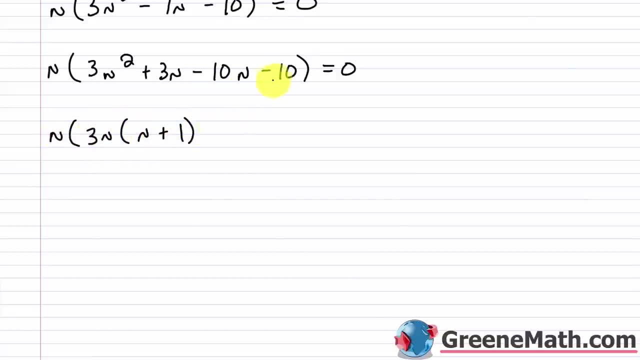 You'll have n plus 1.. And then out of the second group I'm going to put out a negative 10.. I'll have n plus 1. This equals zero. Factor out the common binomial factor of n plus 1.. And you'd have 3n minus 10. 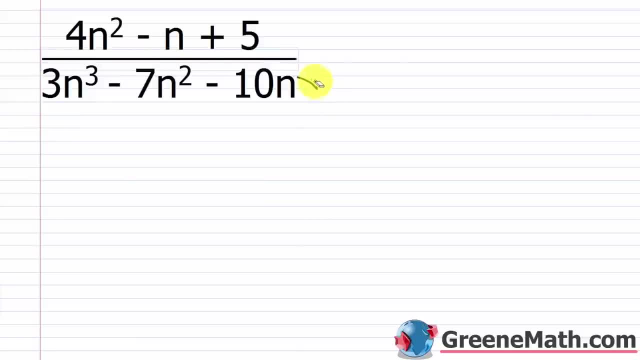 So again, all I want to do is take my denominator, whatever it is, and set it equal to 0 and find out what the restricted values are. So 3n cubed minus 7n squared minus 10n. Again, set this equal to 0. And I'm going to find out what values of n are going to make this denominator 0. And that's, again, what we can't have. Those are the restricted values. So to find out what the restricted values are, I'm going to take my denominator, and to factor this, I notice that I have an n that's common to everything. So let's pull that out to start. So we'd have 3n squared minus 7n minus 10. And this equals 0. And then to factor 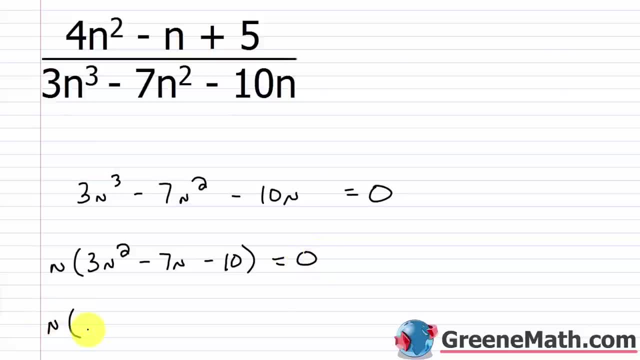 this, I'm going to use the grouping method. And I want you to give me two integers whose product is 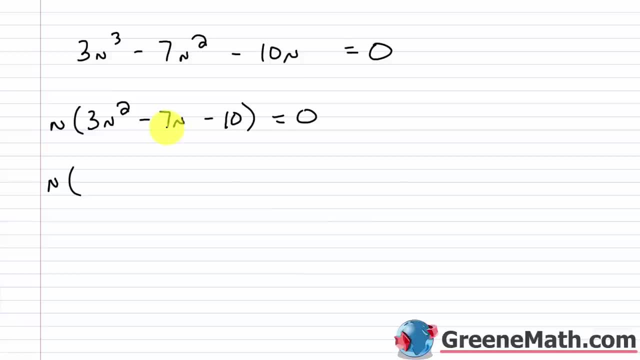 negative 30 and whose sum is negative 7. Well, that's pretty easy. If you think about 10 and 3, 10 times 3 is 30. And then I'm going to use the grouping method. And I want you to give me 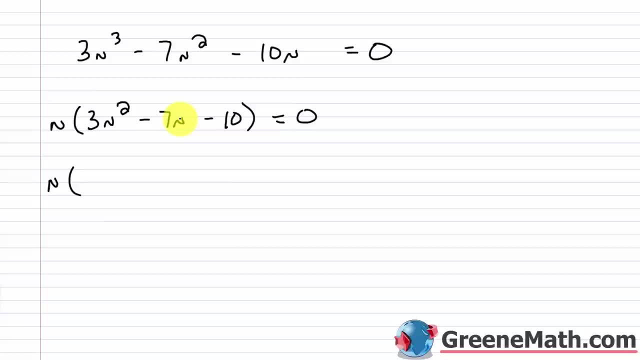 3. And I can manipulate the signs to get to negative 7. So if I think about negative 10 and positive 3, that gives me exactly what I want. So 3n squared. Then I'm going to put plus 3n. 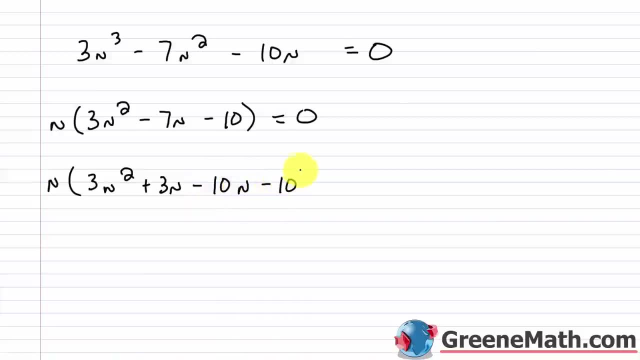 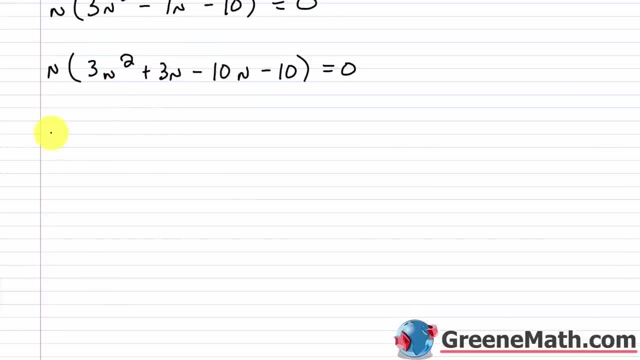 And then minus 10n. And then minus 10. This equals 0. Again, I'm going to be factoring by grouping. So out of this first group, I can pull out a 3n. So I'm going to have n times. Pull out a 3n. You'll have n plus 1. And then out of the second group, I'm going to pull out a negative 10. I'll have n plus 1. This equals 0. Factor out the common binomial factor of n plus 1. And you'd have 3n minus 10 times this n plus 1. This equals 0. And in this case, I have three factors that need to be set 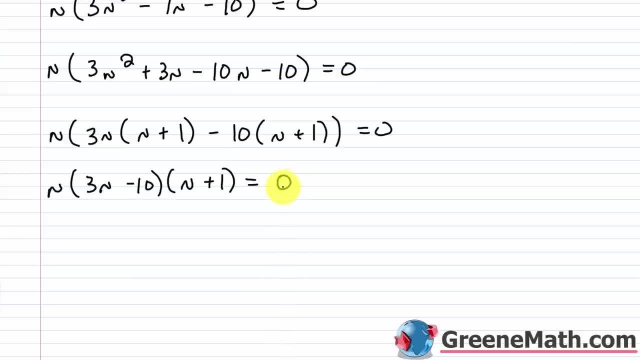 equal to 0. The first one is just n. n equals 0. If n is 0, then the denominator is 0. And you can go up and verify that. 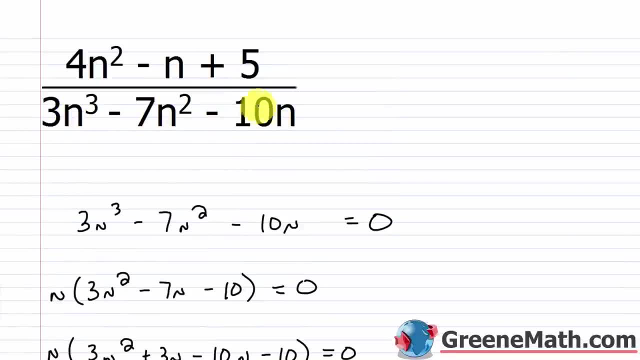 So if I plugged in a 0 here, here, and here, I'd have 0, minus 0, minus 0. That would be 1. 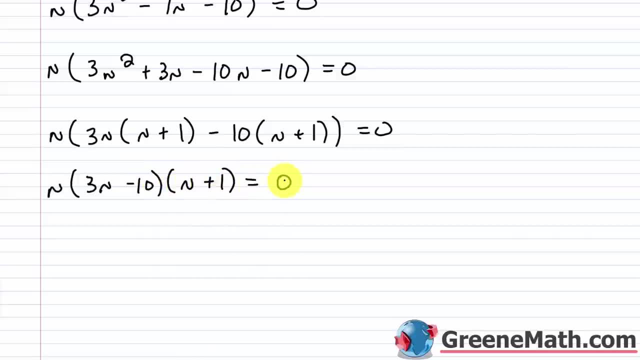 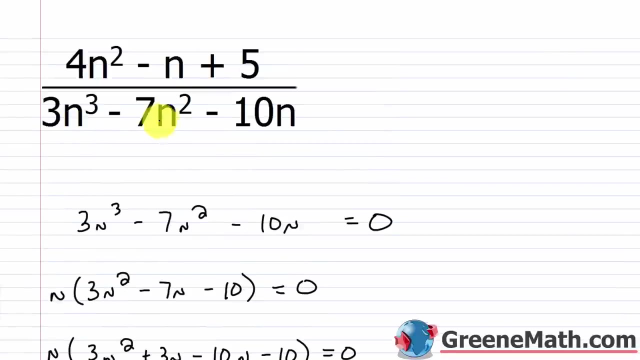 times this: n plus 1.. This equals zero, And in this case I have three factors that need to be set equal to zero. The first one is just n: n equals zero. If n is zero, then the denominator is zero, And you can go up and verify that If I plugged in a zero here, here and here. 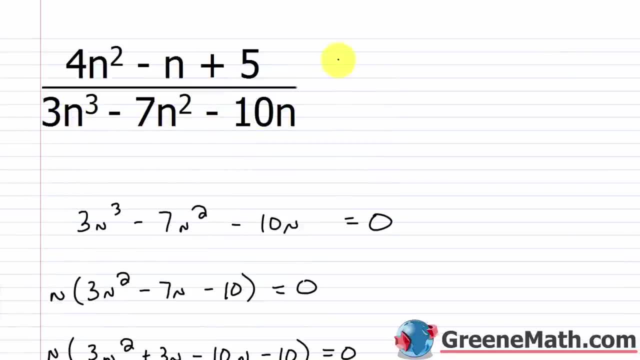 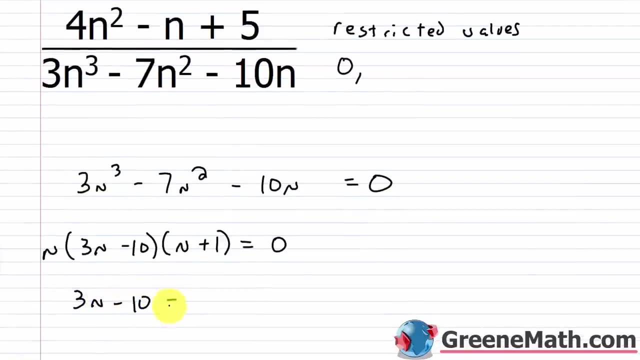 I'd have zero minus zero minus zero. That would be zero. So for your restricted values you'd have zero. So then the other one is: 3n minus 10 equals zero. Set that equal to zero. We add 10 to both sides of the equation And we get 3n is equal to 10.. Divide both sides by 3.. 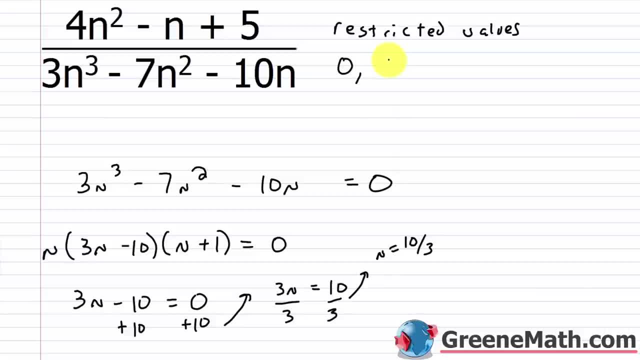 And we're going to get that n is equal to 10 thirds. So another restricted value would be 10 thirds. Provided that it checks out- and it is a solution To this equation- 3n cubed minus 7n, squared minus 10n, equals zero. We'll check that in a minute. 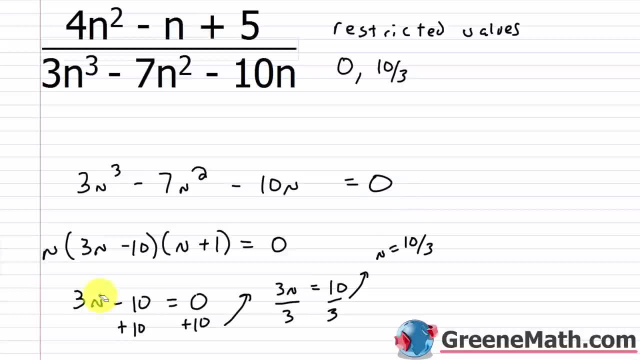 I already know that it works, So we're going to just list it there. And then the last one: we're going to set n plus 1, this factor here equal to zero. n plus 1 equals zero, Of course. 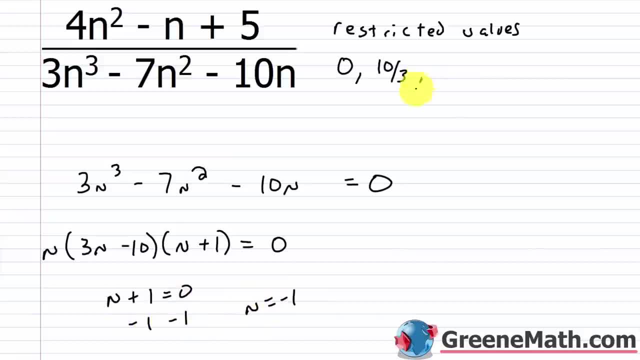 we subtract 1 from each side, We get n equals negative 1.. So we're going to list that as well. So let's check those two real quick And I'll show you that they do in fact work For 10 thirds. it's kind of tedious, But three times 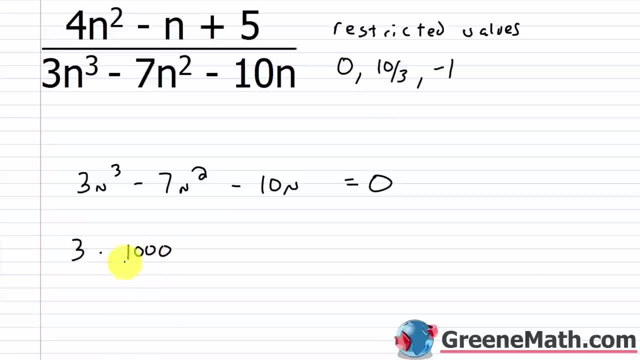 10 thirds cubed would be 1,000 over 27.. Then this would cancel with this and give me a 9 here. So I'd basically have 1,000 over 9.. 1,000 over 9.. And then we'd have minus 7 times 10 thirds. 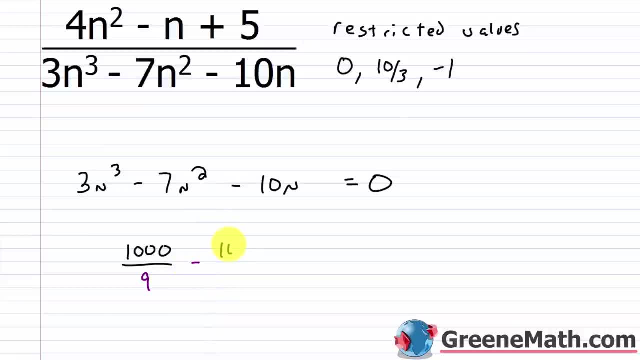 squared 10 squared is 100. So this would be 100. And then 3 squared is 9.. So then, if I multiply that by 7,, how do we get 700 over 9? So 700 over 9.. 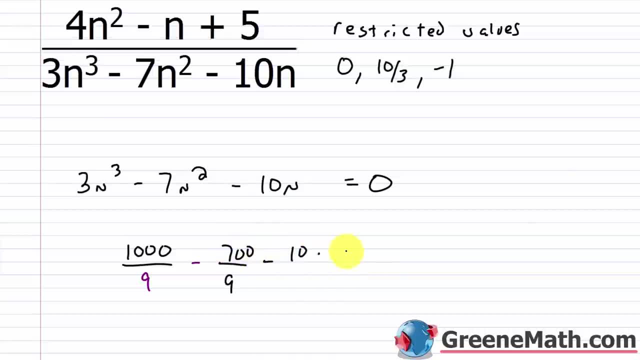 And then minus, we have 10 times 10 thirds. So this would be 100 thirds. Let's go ahead and write that, And this should be equal to zero. Now, if I do 1,000 minus 700, that's 300.. So I'd. 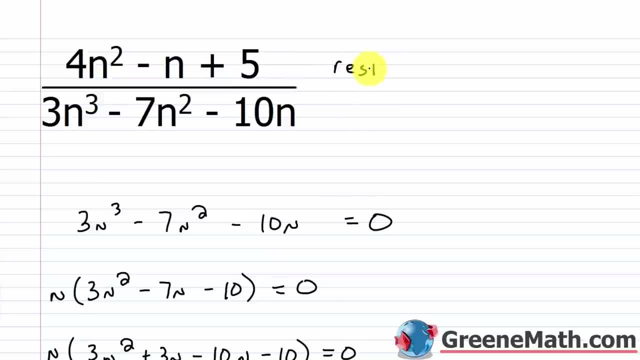 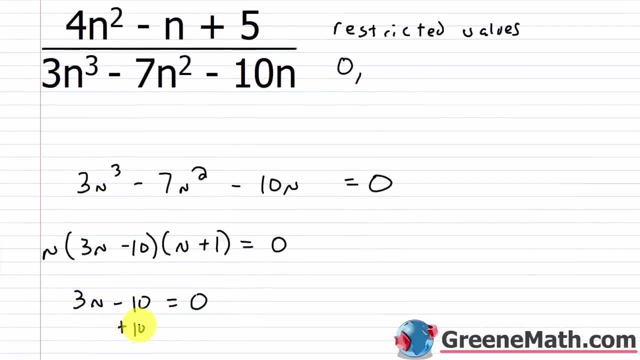 So for your restricted values, you'd have 0. So then the other one is 3n minus 10 equals 0. Set that equals 0. We add 10 to both sides of the equation and we get 3n is equal to 10 . And we're going to get N is equal to 10. Divide both sides by three. And we're going to give that n is equal to 3n. equal to 10 thirds. So another restricted value would be 10 thirds. Provided that it checks out and it is a solution to this equation, three n cubed minus seven n squared minus 10 n equals zero. We'll check that in a minute. I already know that it works. 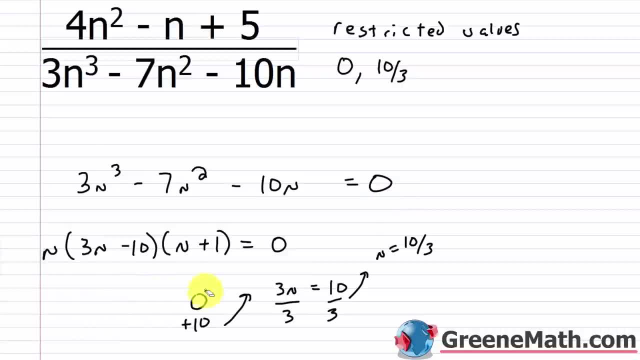 So we're gonna just list it there. And then the last one, we're gonna set n plus one, 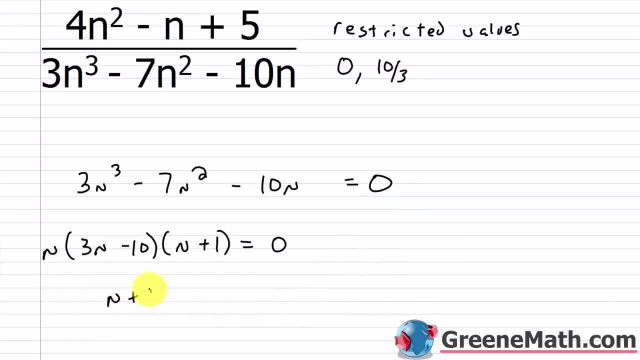 this factor here equal to zero, n plus one equals zero. Of course, we subtract one from each side, we get n equals negative one. 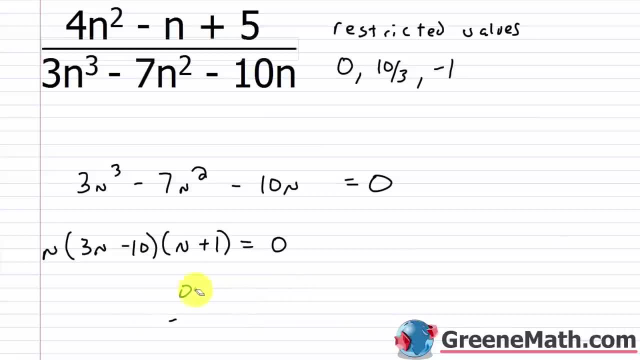 So we're gonna list that as well. So let's check those two real quick and I'll show you that they do in fact work. 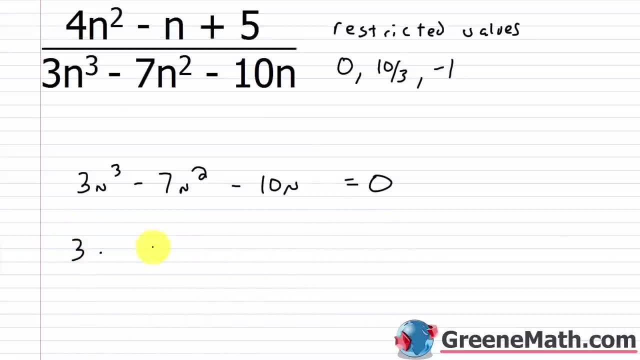 For 10 thirds, it's kind of tedious, but three times 10 thirds cubed would be 1,000 over 27. 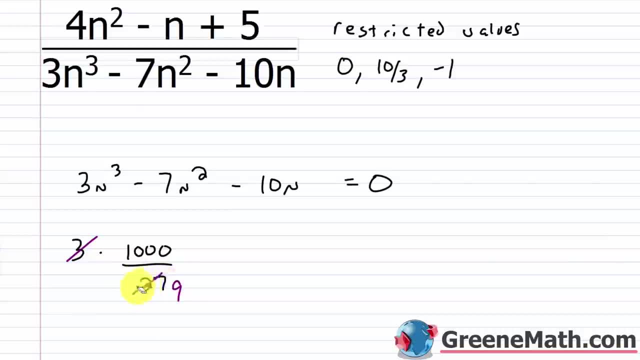 Then this would cancel with this and give me a nine here. So basically I have 1,000 over nine, 1,000 over nine. 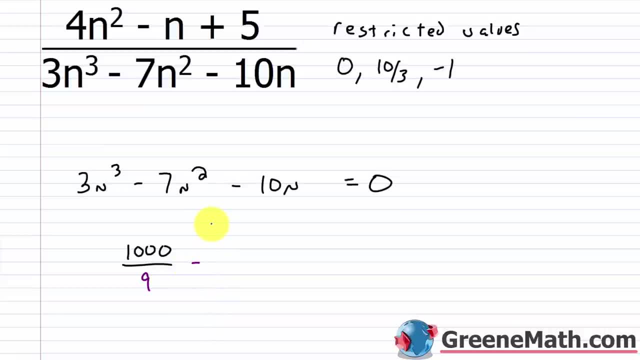 And then we have minus seven times 10 thirds squared. 10 squared is 100, so this would be 100. And then three squared is nine. 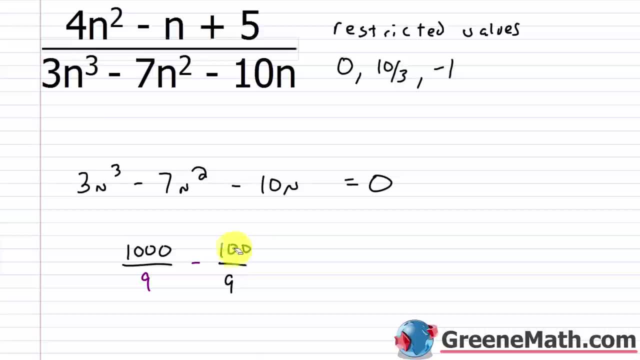 So then if I multiply that by seven, how do we get 700 over nine? So 700 over nine. 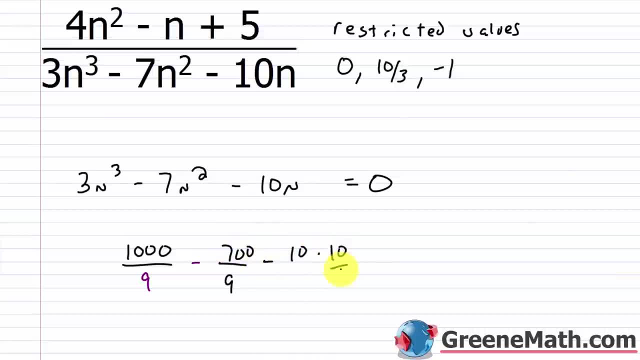 And then minus, we have 10 times 10 thirds. So this would be 100 thirds. Let's go ahead and write that. 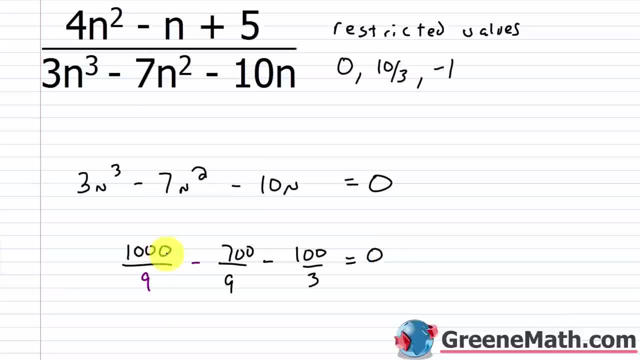 And this should be equal to zero. Now, if I do 1,000 minus 700, that's 300. So I'd have 300 ninths, 300 ninths, which I could simplify because each is divisible by three and write it as 100 thirds. So 100 thirds minus 100 thirds is zero. So that checks out. 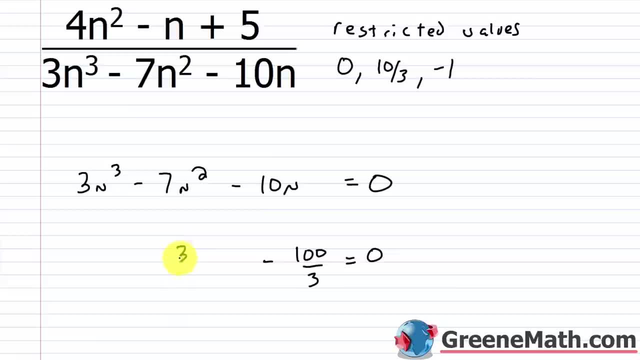 have 300 ninths. 300 ninths, which I could simplify, because each is divisible by 3, and write it as 100 thirds. So 100 thirds minus 100 thirds is zero. So that's checks out All right. So the next one is negative: 1.. So if I plug that in here and here, 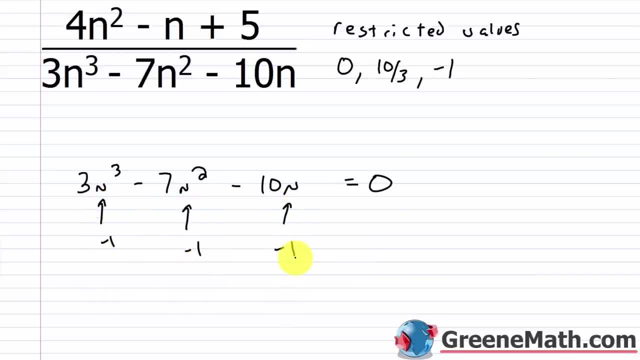 and also here: what am I going to get? Negative 1 cubed is negative 1.. So you'd have negative 3 minus negative 1 squared is 1.. So 1 times 7 is just 7.. Then minus 10 times negative, 1 is negative. 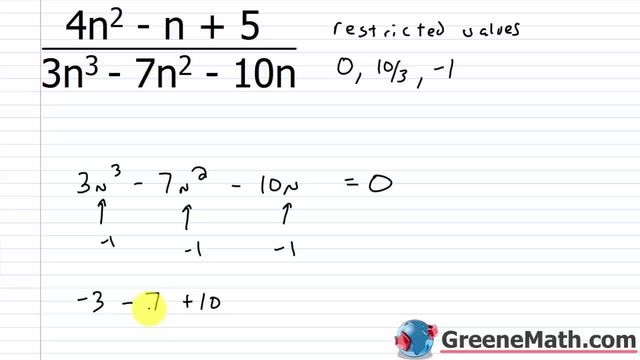 10. You'd have minus a negative 10.. So plus 10.. Negative 3 minus 7 is negative 10.. Negative 10 plus 10 is equal to zero. So this one checks out as well, And so we can say that our restricted values here are 0,, 10 thirds and negative 1.. Right If 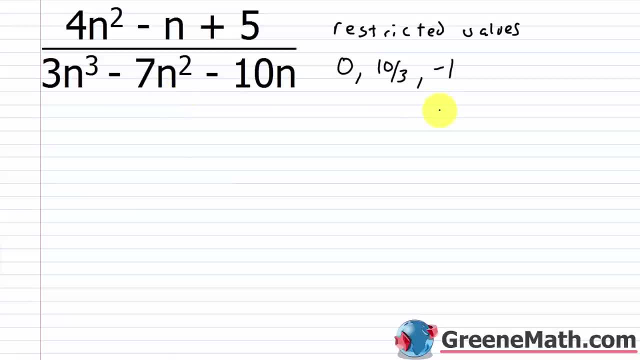 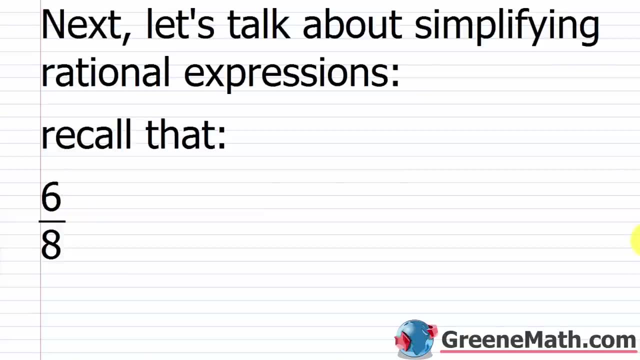 n equals any of those values, you're going to get a denominator of zero, And again that's not allowed. All right, So now let's talk about simplifying rational expressions. So I want you to recall how we go about simplifying a fraction. So if I have something, 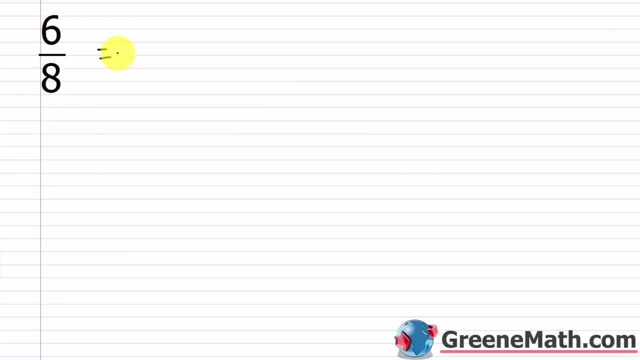 like 6 over 8,. what I'm looking to do is cancel common factors. So 6, I could write as 2 times 3.. 8, I could write as 2 times 4.. But really, if I wanted to really break it down, I could put 2 times 2. 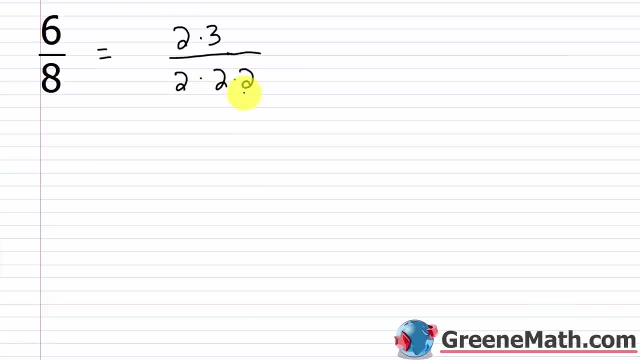 times 2.. It's really only necessary to write 2 times 4, because the greatest common factor between these two is just a 2.. So I cancel that greatest common factor between the two and I end up with 3 over 2 times 2, or I end up with 3 fourths. So now this fraction is considered simplified. 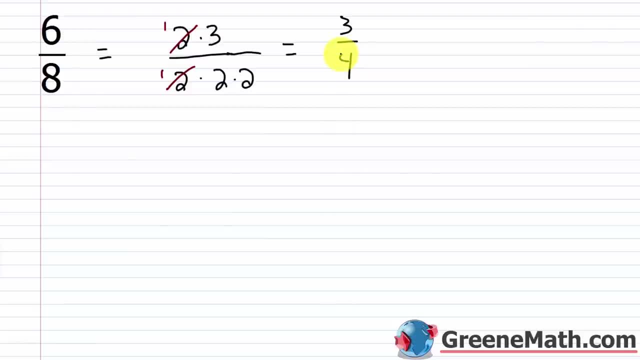 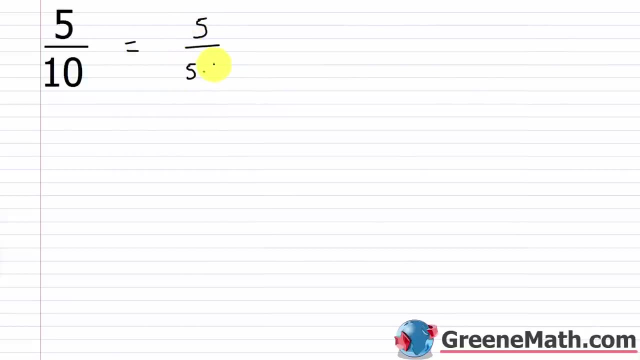 because the greatest common factor is now a 1.. All right, There's nothing else. I can remove Something like 5 tenths. All right, 5 is a prime number, And 10, I can write as 5 times 2.. And so I can cancel this 5 with this 5. And I'll end up. All right, so the next one is negative one. 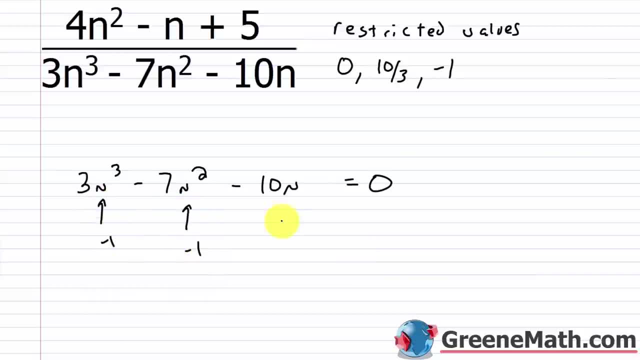 So if I plug that in here and here and also here, what am I gonna get? Negative one cubed is negative one. 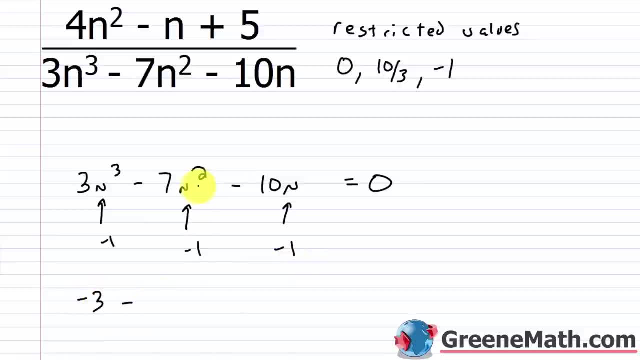 So you'd have negative three minus, negative one squared is one, so one times seven is just seven. Then minus, 10 times negative one is 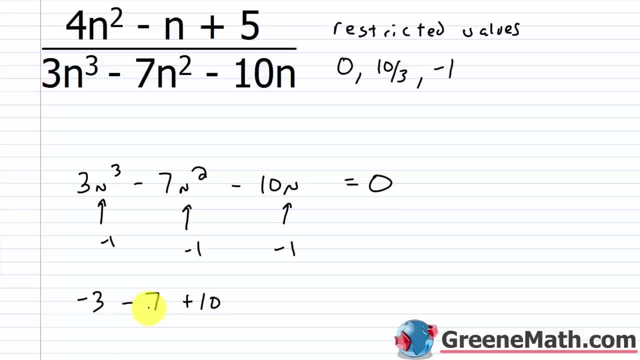 negative 10, you'd have minus a negative 10. So plus 10, negative three minus seven is negative 10, negative 10 plus 10 is equal to zero. So this one checks out as well. And so we can say that 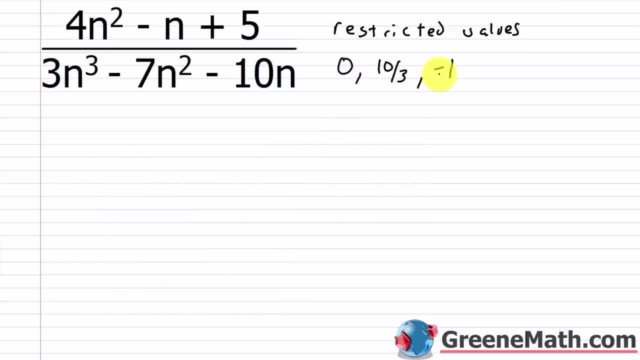 our restricted values here are zero, 10 thirds and negative one, right? If n equals any of those values, you're going to get a denominator of zero. And again, that's not allowed. All right, 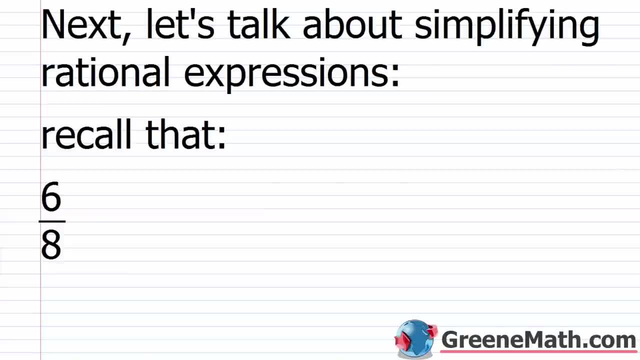 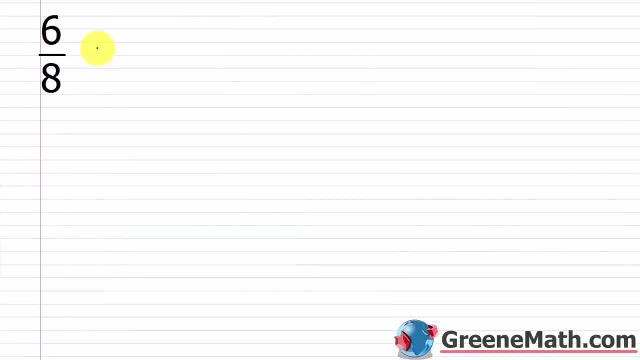 so now let's talk about simplifying rational expressions. So I want you to recall how we go about simplifying a fraction. So if I have something like six over eight, what I'm looking 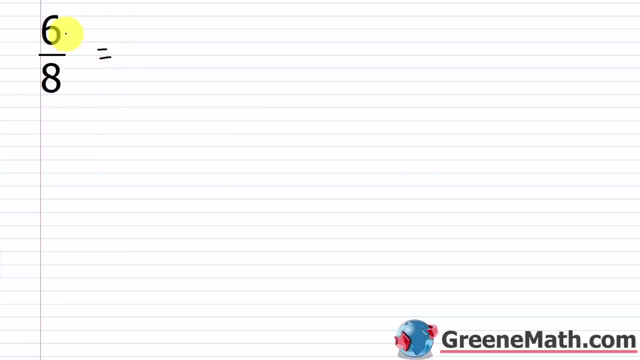 to do is cancel common factors. So six, I could write as two times three. Eight, I could write as two times four. But really, if I wanted to really break it down, I could write two times two times two. It's really only necessary to write two times four because the greatest common factor between these two is just a two. So I cancel that greatest common factor between the two, and I end up with, 3 over 2 times 2, or I end up with 3 fourths. So now, this fraction is considered simplified because the greatest common factor is now a 1. There's nothing else I can remove. 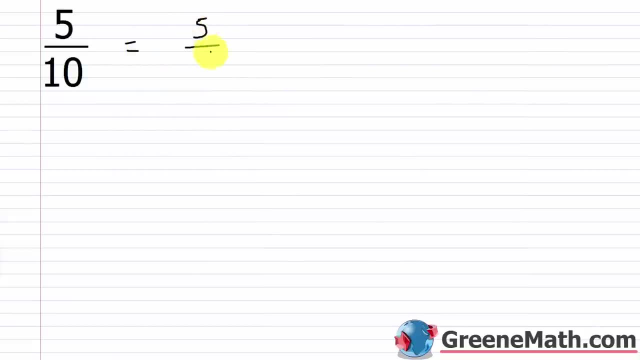 Something like 5 tenths. 5 is a prime number, and 10 I can write as 5 times 2, and so I can cancel this 5 with 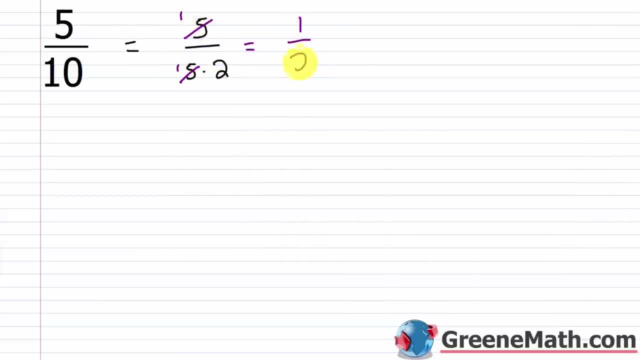 this 5, and I'll end up with 1 over 2, or 1 half. 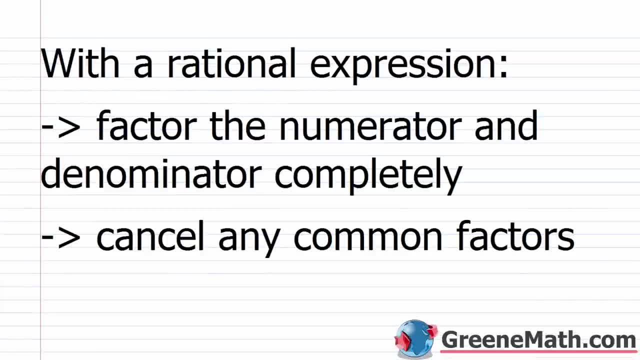 with 1 over 2, or 1 half. So, with a rational expression, we're going to factor the numerator and denominator completely, just like we did with the fraction, And we're going to cancel any common factors. All right, So let's take a look at the first problem here, And we're going to start out. 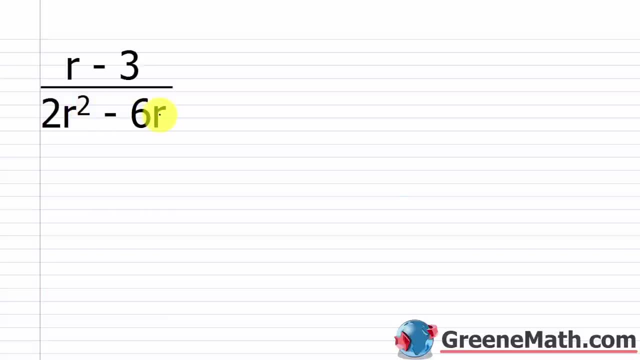 with 2r squared minus 6r. So again, the first thing you want to do, just like when you work with fractions and you were told to simplify them- you want to factor your numerator and denominator completely. So in the numerator, r minus 3 is not going to factor, So you're just 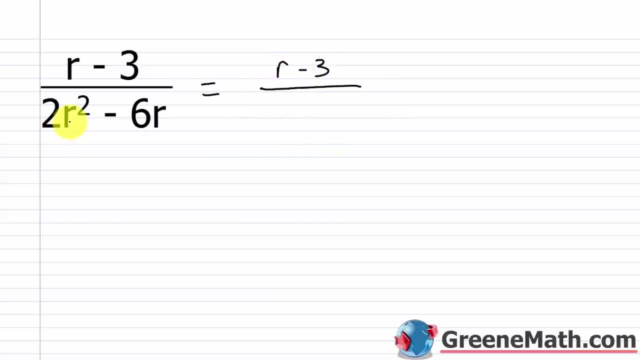 going to leave that as it is In the denominator, the 2r squared minus 6r. I can pull a 2r out and set it out in front of some parentheses, because that's common to each, And then inside of the. 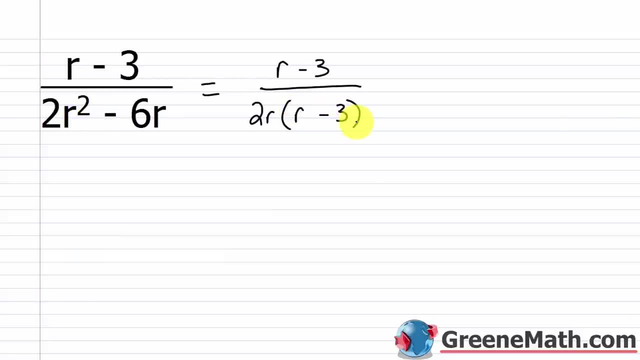 parentheses, I would have an r minus a 3. So now, what do I have that's common? I have r minus 3 here and r minus 3 here, So it's common to both numerator and denominator. And when that happens. 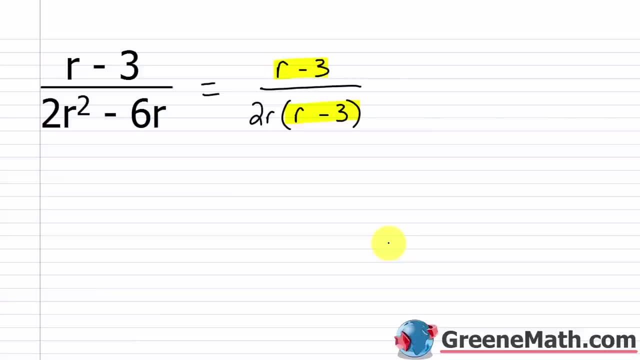 you can cancel it. Now, when you first start doing this, you might be like, well, how do I go about doing that? Remember, these are factors. So this is multiplication here, This is a factor And this is a factor. You might say, well, that's not a factor up here. Well, yeah, I could write it. 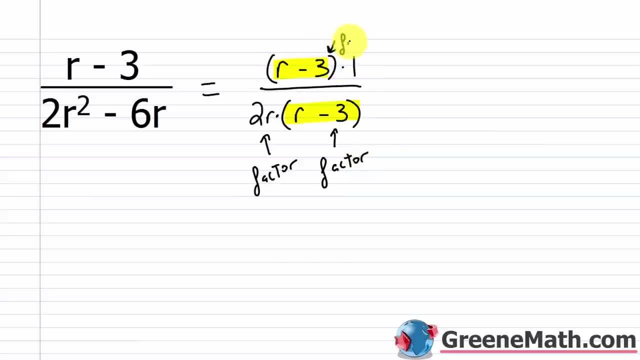 times 1.. And then again I could do the same thing. I could say: this is a factor and this is a factor. So now it's completely clear that I can cancel this factor of r minus 3 with this factor of r minus 3.. And the simplified version is just going to be a 1 in the numerator. That's what's. 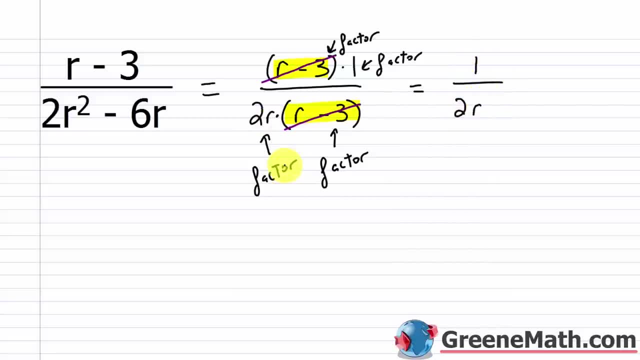 left over a 2r in the denominator. That's what's left there, So 1 over 2r. If we want to just quickly refer back to an example, we did with fractions, we looked at 5 over 2r. We looked at. 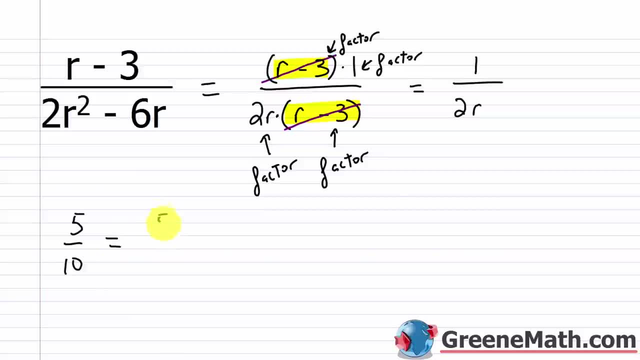 10. 5 doesn't factor. It's a prime number. So we could write 5 times 1 if we wanted to over 10. We write as 5 times 2.. So what am I doing? I'm canceling a common factor of 5. And I'm left. 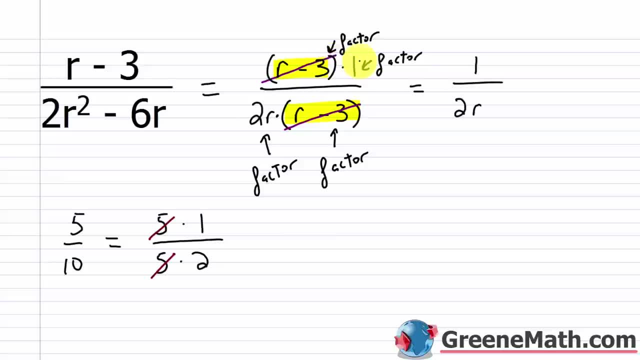 with 1 over 2.. Same thing I did here. I canceled a common factor of r minus 3.. That's all we're doing here. It's not more difficult. You just need to realize one key thing, And I'm going to. 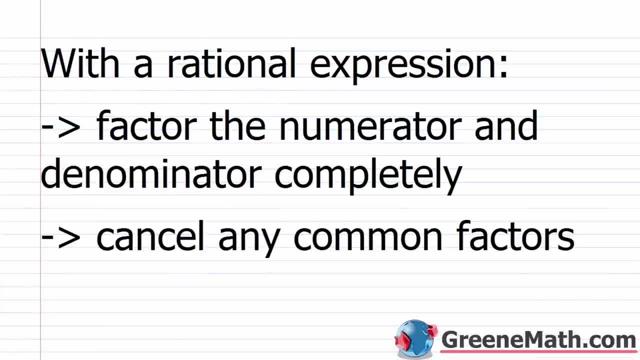 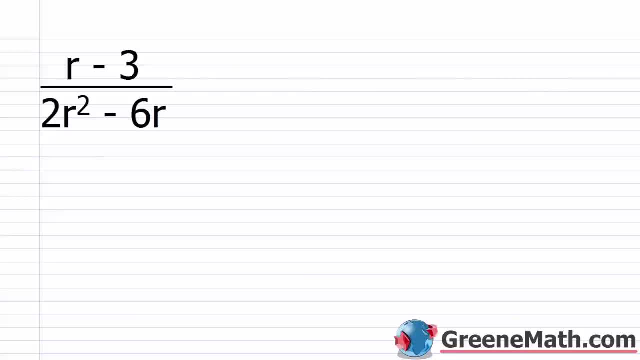 So with a rational expression, we're going to factor the numerator and denominator completely, just like we did with the fraction, and we're going to cancel any common factors. All right, so let's take a look at the first problem here, and we're going to start out with r minus 3 over 2r squared minus 6r. 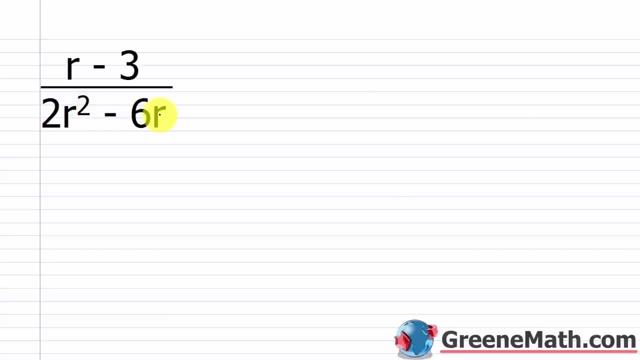 So again, the first thing you want to do, just like when you worked with fractions and you were told to simplify them, you want to factor your numerator and denominator completely. 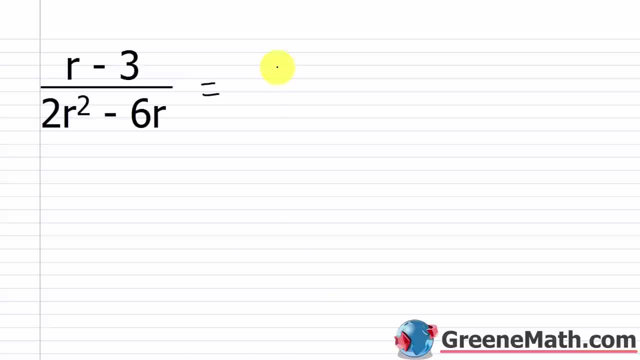 So in the numerator, r minus 3 is not going to factor. So you're just going to leave that as it is. 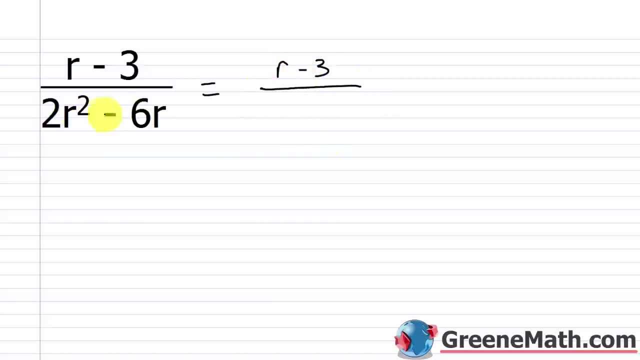 In the denominator, the 2r squared minus 6r, I can pull a 2r out and set it out in front of some parentheses, because that's common to each, and then inside of the parentheses I would have an r minus a 3. 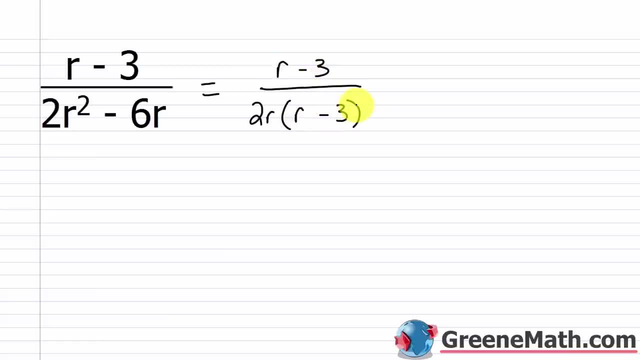 So now what do I have that's common? I have r minus 3 here, and r minus 3 here. So it's common to both numerator and denominator, and when that happens, you can cancel it. Now, when you first start doing this, you want to do this. When you first start doing this, you might be like, well, how do I go about doing it? 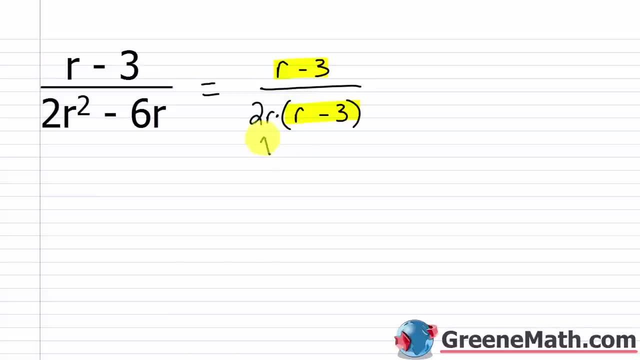 Remember, these are factors. So this is multiplication here. This is a factor, and this is a factor. You might say, well, that's not a factor up here. Well, yeah, I could write it as times 1, and then again, I could do the same thing. I could say this is a factor, and this is a factor. So now it's completely clear that I can cancel this factor of r minus 3 with this factor of r minus 3. 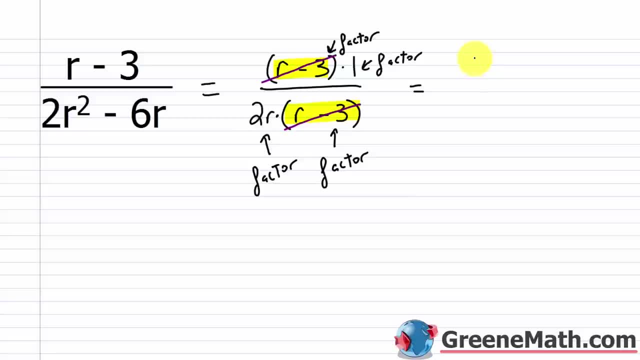 And the simplified version is just going to be a 1 in the numerator, that's what's left, over a 2r in the denominator, that's what's left there, so 1 over 2r. 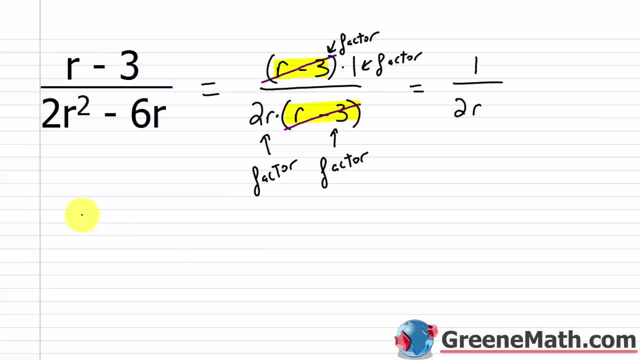 If we want to just quickly refer back to an example we did with fractions, we looked at 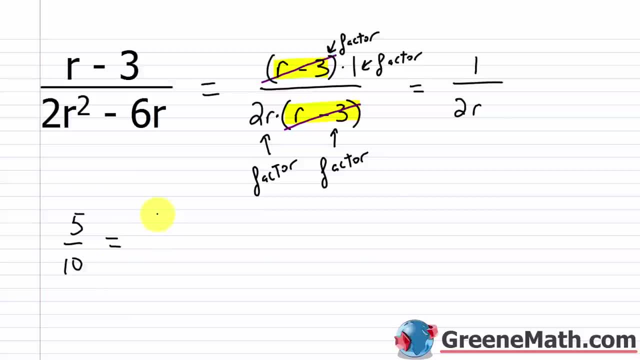 5 over 10, five dozen factors, a prime number. So we could write 5 times 1 if we wanted to, over 10 we write as 5 times 2. So what am I doing? I'm canceling a common factor of 5, and I'm left with 1 over 2. Same thing I did here. 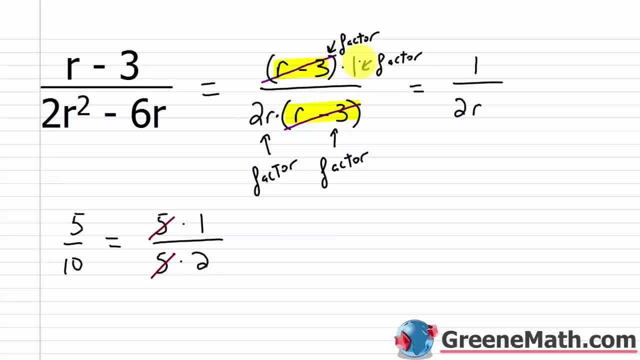 Canceled a common factor of r minus 3. That's all we're doing here. It's not more difficult. 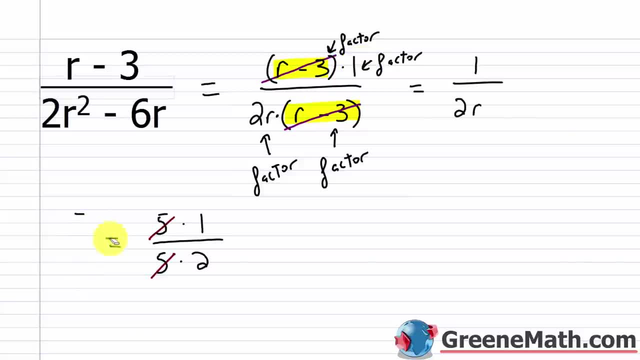 You just need to realize one key thing, and I'm going to explain that to you right now. This is what trips up a lot of students. If I have something like, let's say, 2r plus 1 over 2, can I cancel this 2 with this 2? No, I cannot. 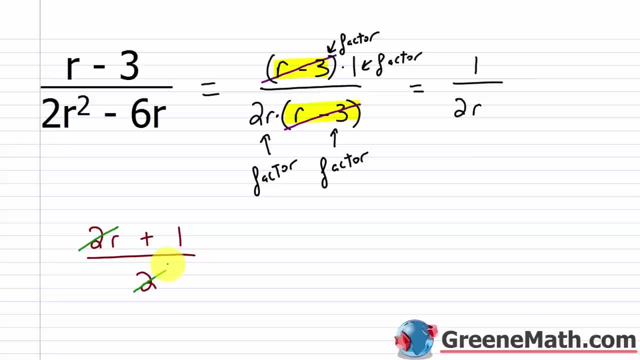 This is the most common mistake I see when we first start working with rational equations. It's the most common mistake I see when we first start working with rational equations. It's the most common mistake I see when we first start working with rational equations. 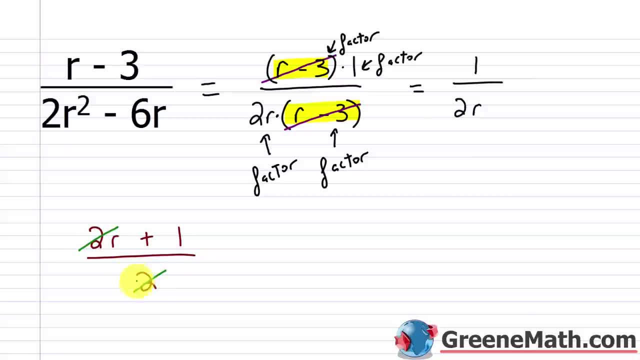 It's the most common mistake I see when we first start working with rational equations. For some reason, students start thinking that they can just cancel, or they see something 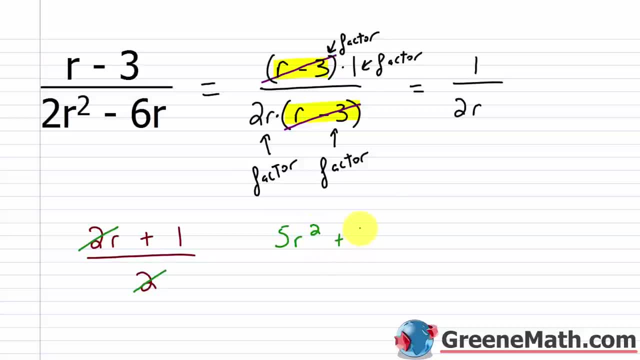 like, okay, I have 5r squared plus 3 over 15. Well, they'll go through and say, okay, well, some of them will cancel this 5 with the 15 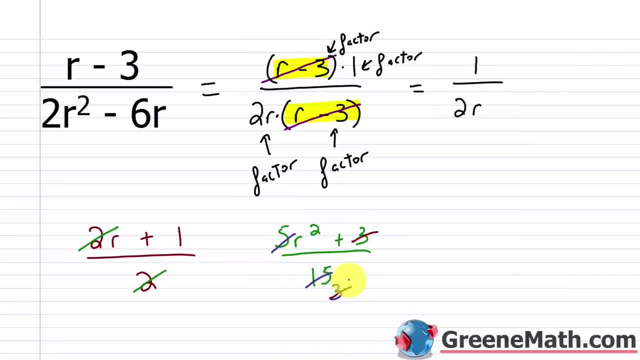 and put a 3, and then they'll say, okay, I can also cancel this 3 with this 3. No, you cannot do that. These are both wrong. These are wrong. Why are they wrong? 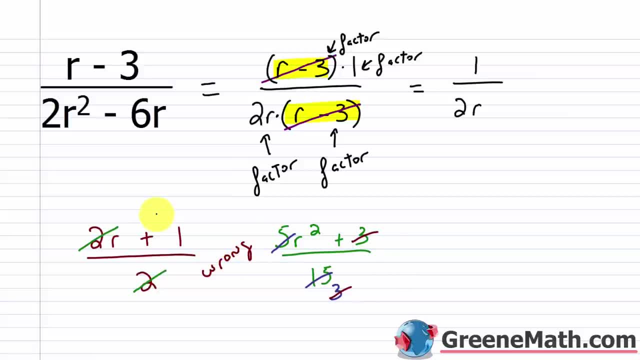 Well, because I'm canceling common factors. This is just addition here. This is addition. It's not multiplication. This is addition. It's not multiplication. 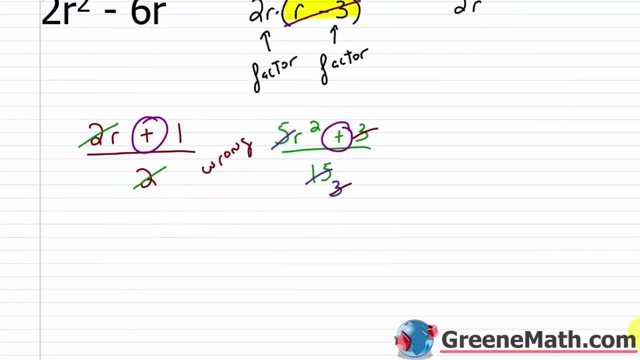 I can't cancel anything. Where I can cancel, if I saw something like, let's say, 2r plus 2 over 2, and I factored my numerator. I notice that there's a 2 that's common to each term there. 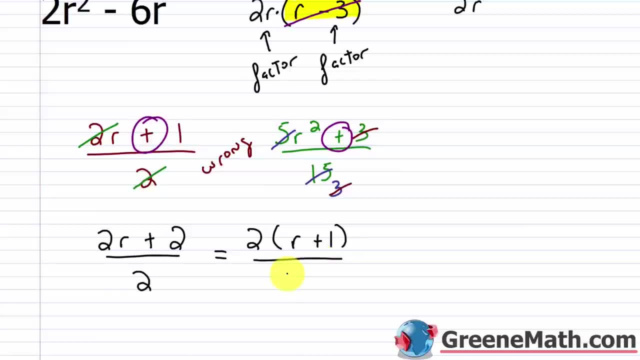 So I write this as 2 times the quantity r plus 1 over 2. Now I have multiplication. 2 is a factor, and the quantity r plus 1 is a factor. 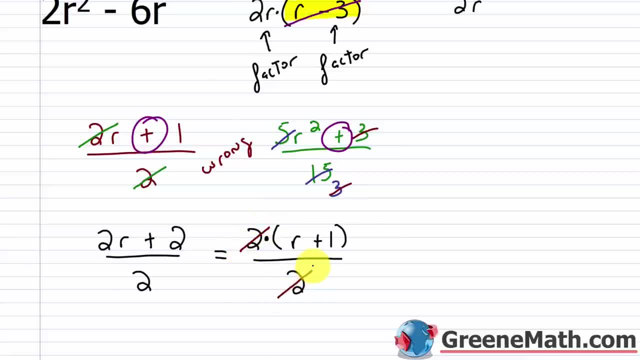 So I can cancel this factor of 2 with this factor of 2. Again, I could write this 2 as 2 times 1. So now this simplifies to what? 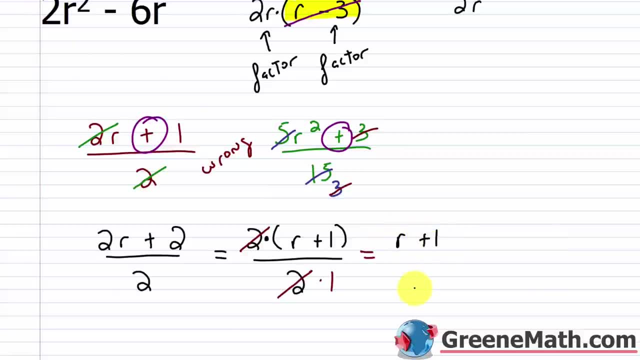 It simplifies to r plus 1 over 1, or really just r plus 1. So we're looking to cancel common factors, okay? Please don't make this mistake. 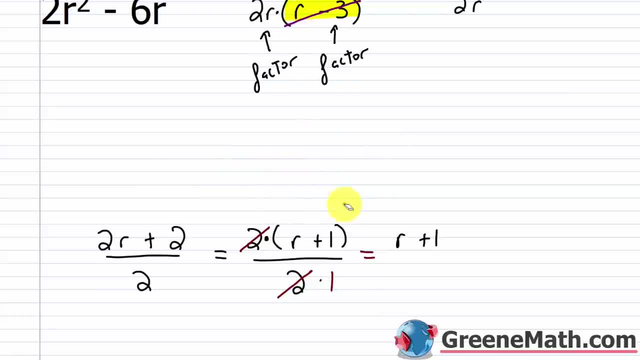 The way you want to remember it, if you want a generic example, it's in a lot of textbooks. 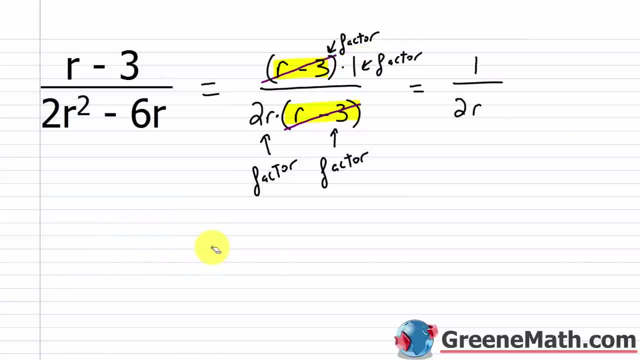 explain that to you right now. This is what trips up a lot of students. If I have something like, let's say, 2r plus 1 over 2. Can I cancel this 2 with this 2? No, I cannot. This is the most common mistake. 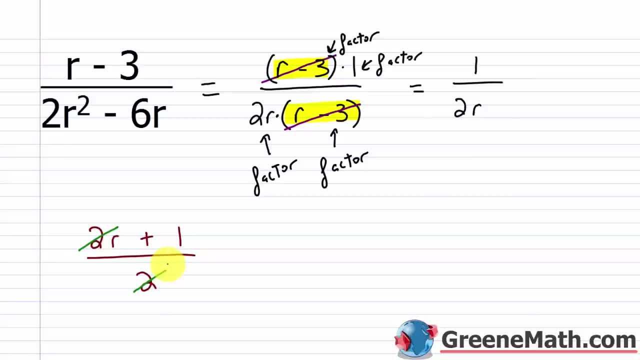 I see, when we first start working with rational expressions, For some reason students start thinking that they could just cancel. Or they see something like: OK, I have 5r squared plus 3 over 15.. Well, they'll go through and say, OK. well, some of them will cancel this 5 with the. 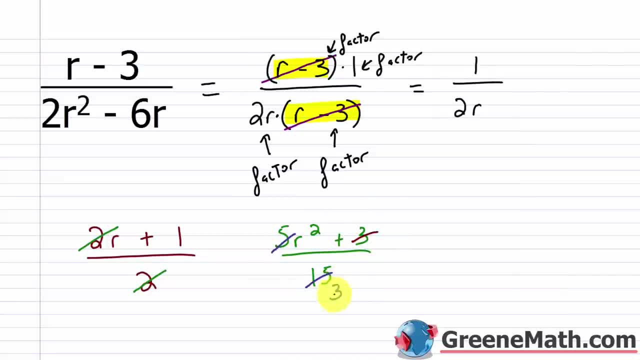 15 and put a 3.. And then they'll say: OK, I can also cancel this 3 with this 3.. No, you cannot do that. These are both wrong. These are wrong. Why are they wrong? Well, because I'm canceling common factors: This: 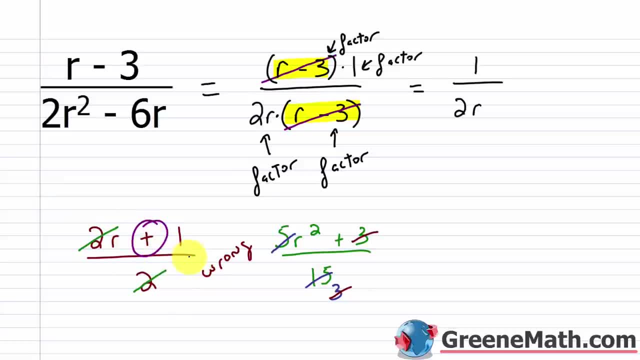 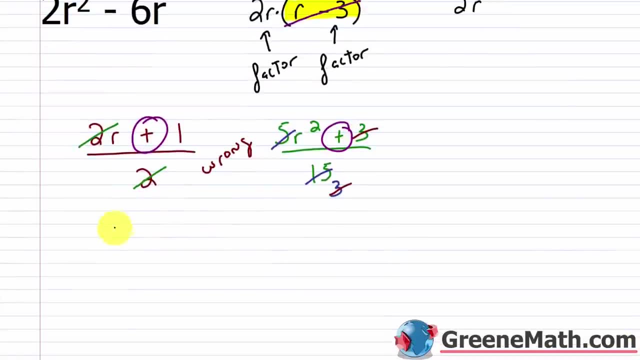 is just addition here. This is addition, It's not multiplication. This is addition, It's not multiplication. I can't cancel anything Where I can cancel. if I saw something like, let's say, 2r plus 2 over 2. And I factored my numerator. 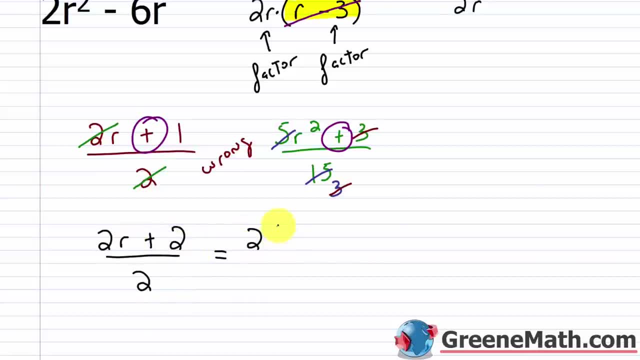 Notice that there's a 2. that's common to each term there, So I write this as 2 times the quantity r plus 1 over 2.. Now I have multiplication. 2 is a factor And the quantity r plus 1 is a factor. 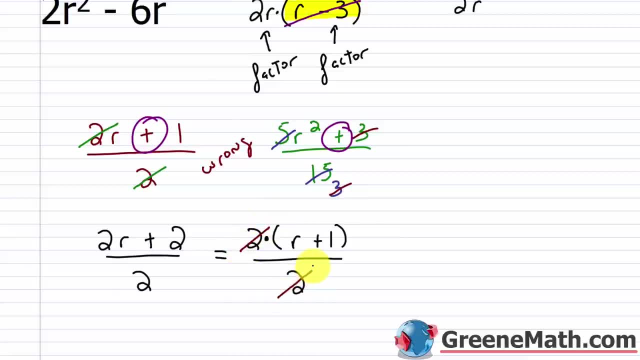 So I can cancel this factor of 2 with this factor of 2.. Again, I could write this 2 as 2 times 1.. So now this simplifies to what It simplifies to r plus 1 over 1, or really just r plus 1.. 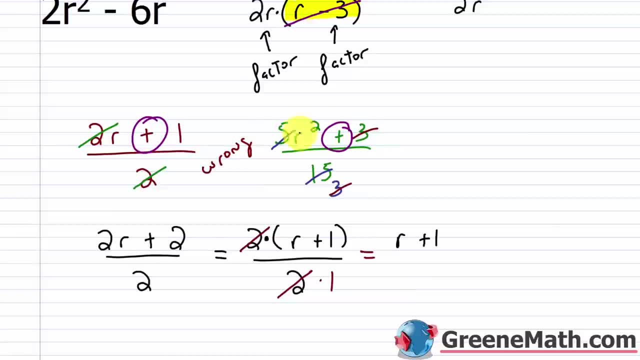 So we're looking to cancel common factors. OK, Let's take this mistake The way you want to remember it. if you want a generic example, it's in a lot of textbooks. You might see something like: a plus b over a is not equal. 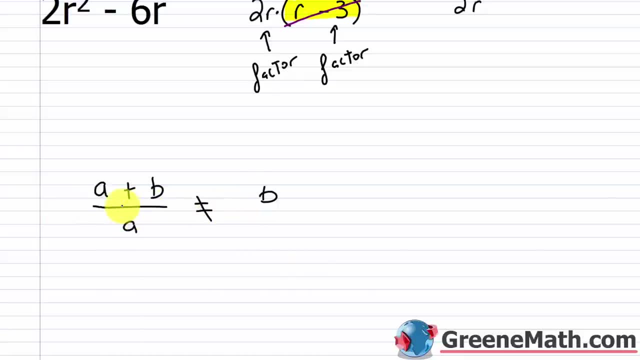 to b, Because a lot of students will see that and say, OK, well, there's an a here and an a here, So I can cancel this with this And I'm just left with b. That's wrong Again. if I had something like a plus ab over a, well then I. 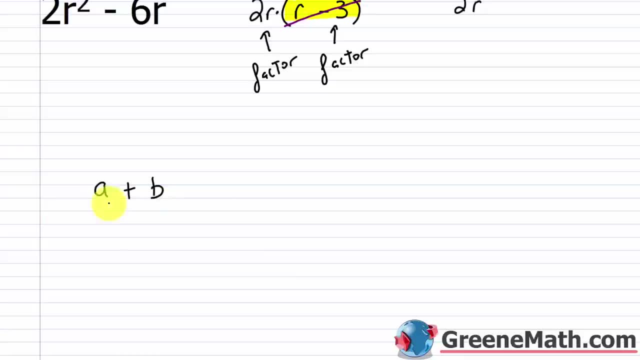 You might see something like, you know, a plus b over a. Okay. 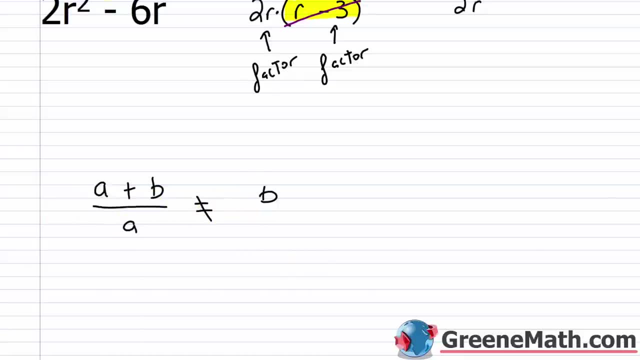 It's not equal to b, because a lot of students will see that and say, okay, well, there's an a here and an a here, so I can cancel this with this, and I'm just left with b. That's wrong. 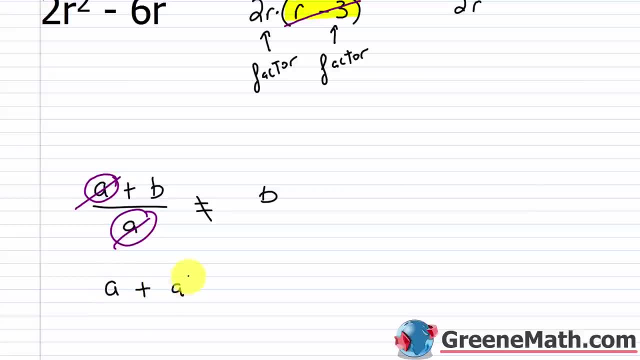 Again, if I had something like a plus ab over a, well, then I could factor the numerator as a times the quantity 1 plus b. And you see what I did there. 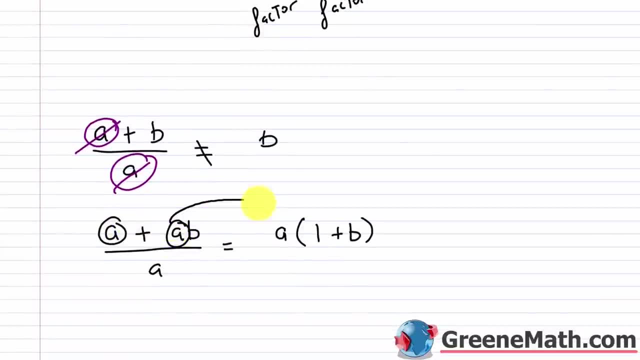 I had an a here and an a here, and I pulled it out and put it outside of the parentheses. And so a times 1 would be a, that would give me that back, a times b would be ab. So all I did was factor that a out and put this over a. And now in this particular case, again, these are factors now. A is a factor, the quantity 1 plus b is a factor, and so I can cancel common factors. So very, very important that you understand that. All right. 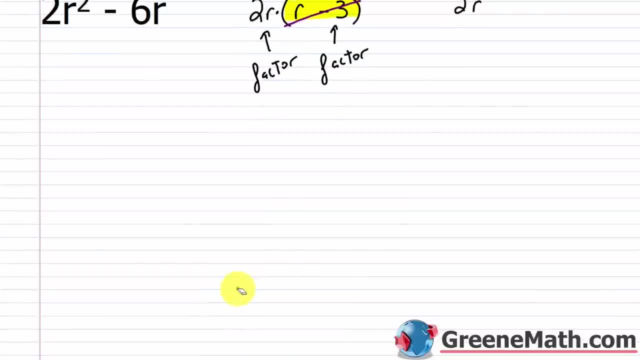 Now, one other thing that I want to address before we kind of move on, in a lot of cases, you're going to get a joint question. 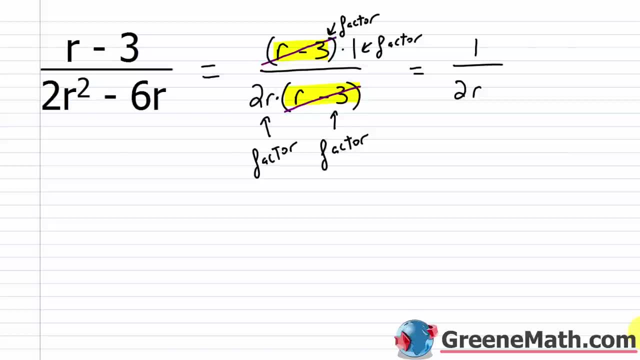 So you might be asked to state the restricted values and to simplify. So let's say you go through, and let me kind of erase all this kind of work that we did. Let's say you go through and you identify that this simplifies to this, and you say, okay, I'm ready to state my restricted values now. 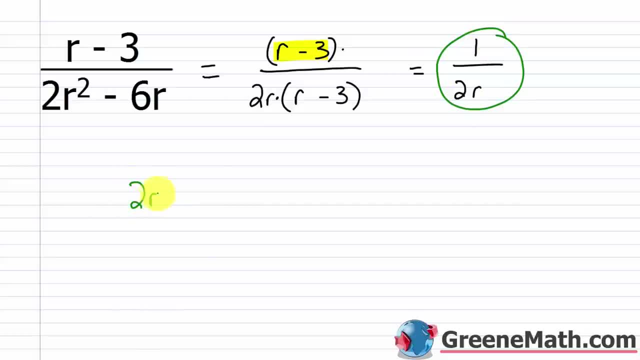 So I look at the denominator, it's 2r. So I say, okay, 2r equals 0, solve that for r, divide both sides by 2. I get r equals 0, and I say, okay, r cannot be 0 because that makes the denominator 0. Well, yeah, that's right, but you're only partially correct. The original denominator is what you have to look at. 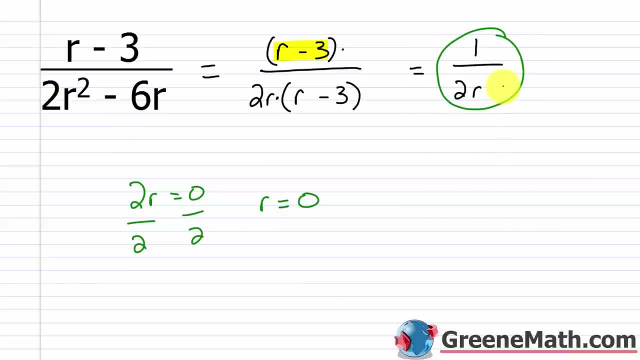 So although the simplified version would be defined for r equals 3, the original is not. So although these two are equal in the traditional sense where we say, okay, we can simplify this and they're equal, you kind of have to put a side note and say it's still not defined for r equals 3. Okay. 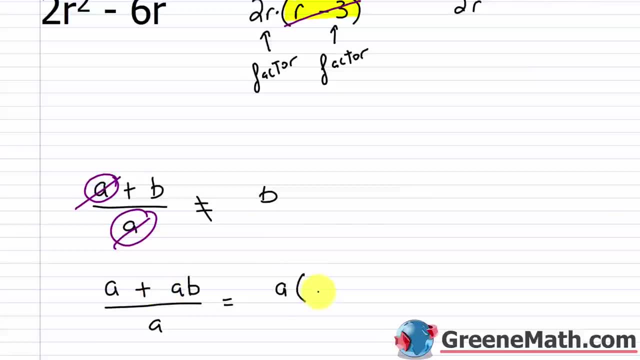 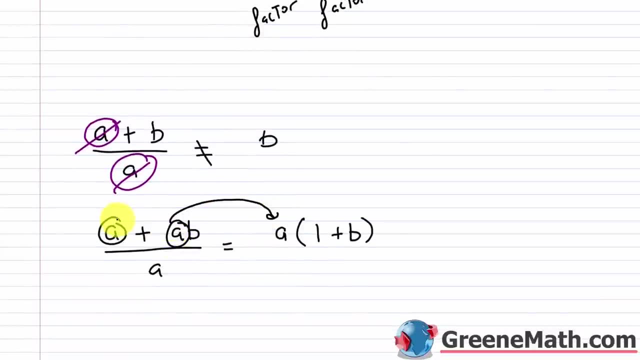 could factor the numerator as A times the quantity 1 plus b. And you see what I did there. I had an a here and an a here And I pulled it out and put it outside of the parentheses And so A times 1 would be A. that would give me that back. A times B would be ab. 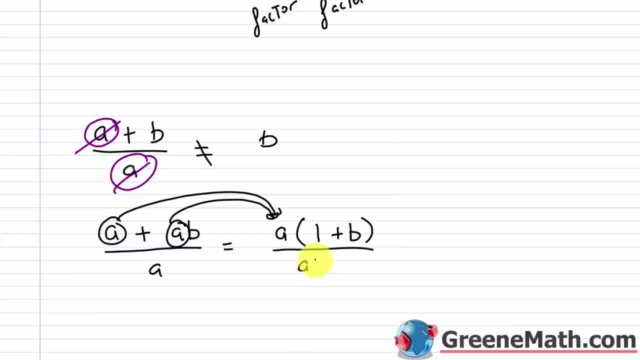 So all I did was factor that a out and put this over a. And now, in this particular case, again, these are factors. now A is a factor, the quantity 1 plus B is a factor, And so I can cancel common factors. So very, very important that you understand that. All right. Now one other thing. 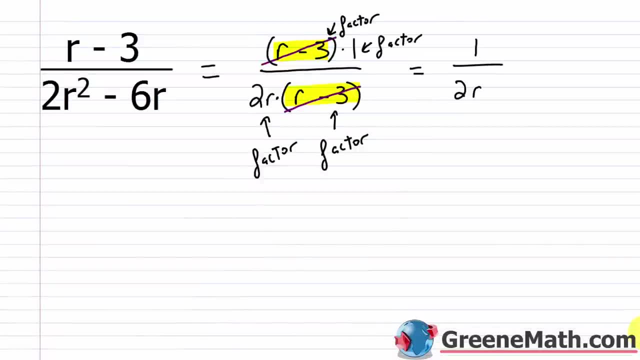 that I want to address before we kind of move on. in a lot of cases you're going to get a joint question, So you might be asked to state the restricted values and to simplify. So let's say you go through and let me kind of erase all this kind of work that we did. Let's say you go through. 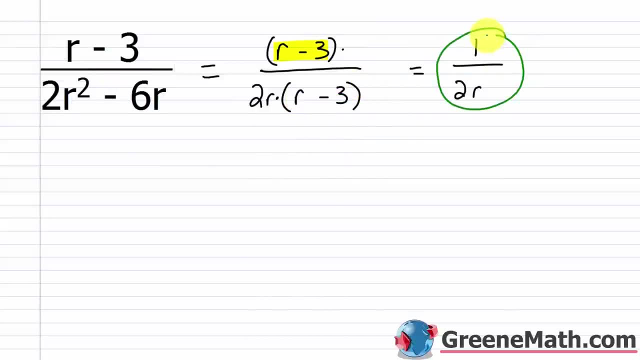 and you identify that. this simplifies to this. You say, okay, I'm ready to state my restricted values now. So I look at the denominator: It's 2r. So I say, okay, 2r equals 0.. Solve that for r. 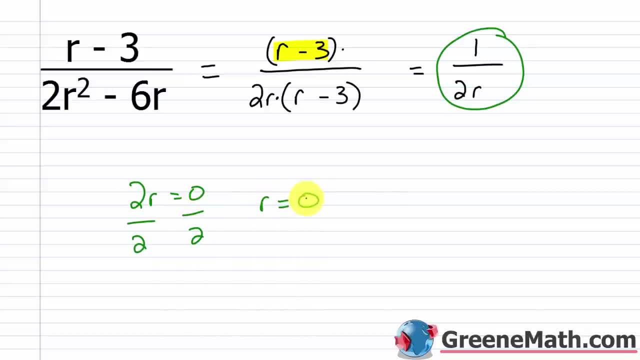 Divide both sides by 2. I get r equals 0. And I say, okay, r cannot be 0, because that makes the denominator 0.. Well, yeah, that's right, But you're only partially correct. The original denominator. 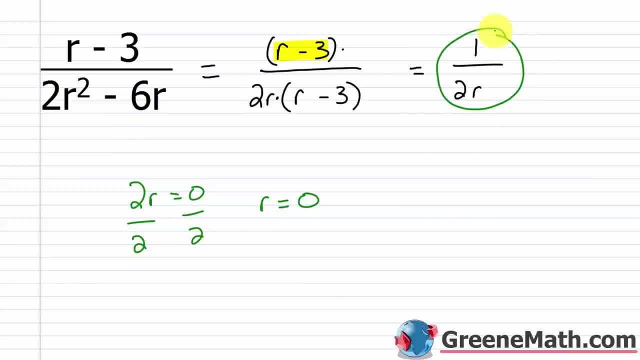 is what you have to look at. So, although the simplified version would be defined for, r equals 3, the original is not, So I'm going to. So I'm going to, although these two are equal in the traditional sense, where we say, okay, we can simplify this. 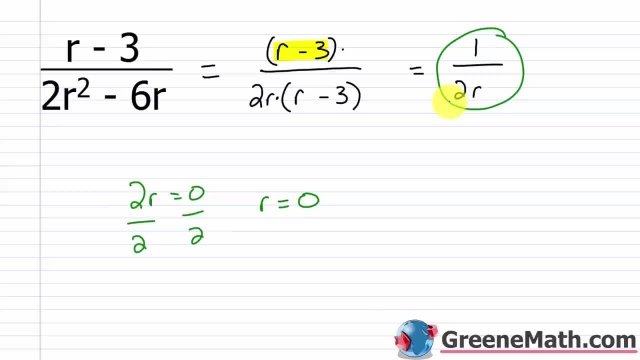 and they're equal. you kind of have to put a side note and say it's still not defined for r equals three. Because in this original one, if I look at this factor denominator, which is this right here, I have this factor: r minus three equals zero. If I add three to both sides, r equals three there. 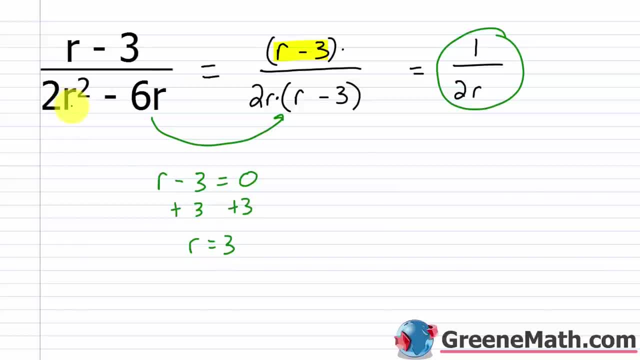 So if I plug a three into the original denominator, I would get a value of zero. Since we started out with that rational expression, we really can't say that these two are equal, because this one is not defined when r is three. This one is right if we just look at one. 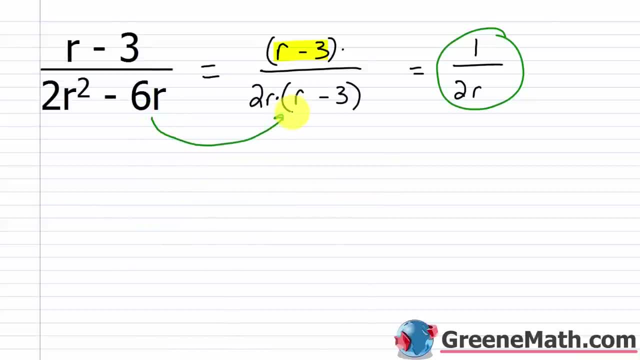 So for example, if I look at this factor denominator, which is this right here, I have this factor r minus 3 equals 0. If I add 3 to both sides, r equals 3 there. So if I plug a 3 into the original denominator, I would get a value of 0. 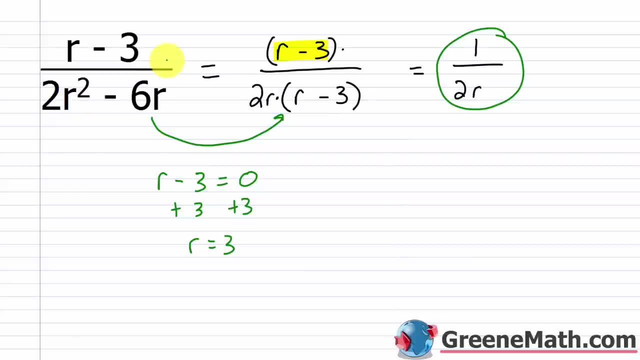 Since we started out with that rational expression, we really can't say that these two are equal because this one is not defined when r is 3. 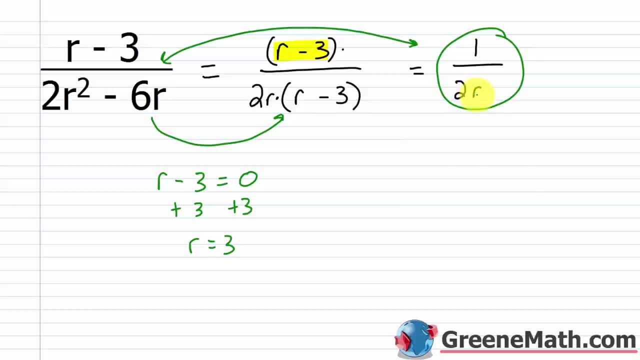 If I plug in 1 over 2r, I can plug in a 3, right? So 2 times 3 is 6, I'd have 1 over 6. So that's where students get confused. 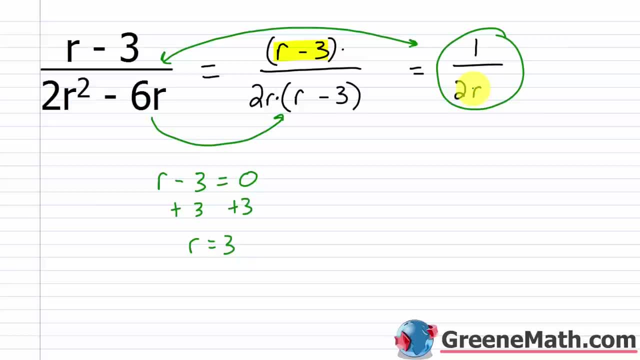 So you almost need like a side note there to kind of explain that and say, well, they are equal, but not if r is equal to 3. And the way you say that is you look at your original rational expression and you look at that denominator to give you your proper restricted values. Okay. So if you stick with the original denominator, you're always going to be good to go. Okay. All right. 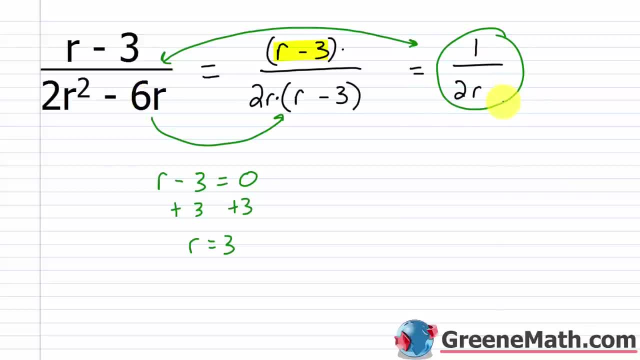 So let's take a look at the simplified one because you might not list all of them. All right. Let's take a look at it all. So we have 15b over 9b squared plus 15. 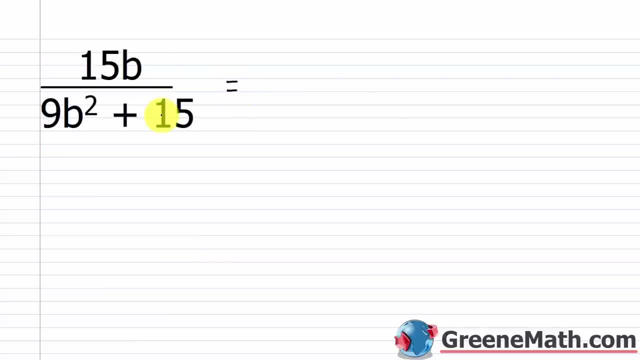 So what can I do here? Again, I want to factor the numerator, denominator. 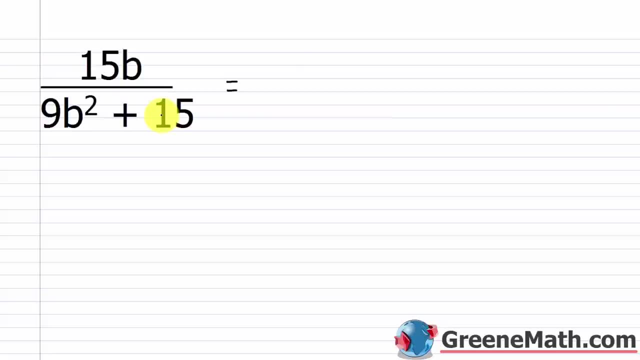 And for the numerator, I know I could break 15 into 5 times 3. So let's go ahead and just do that. 5 times 3. And then I have that b, so times b. 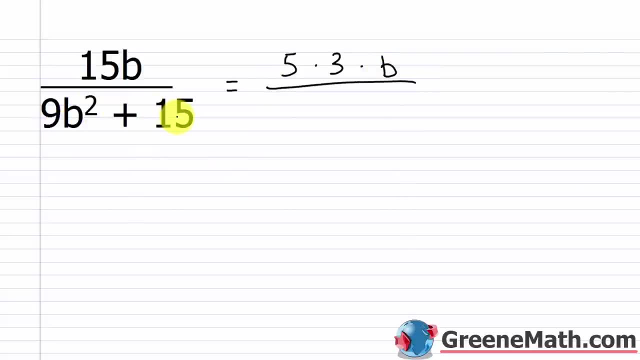 In the denominator, I have 9b squared plus 15. So what's common? The term there would be a 3. Right? So if I pulled a 3 out, I would have what? I'd have 3b squared plus 5. 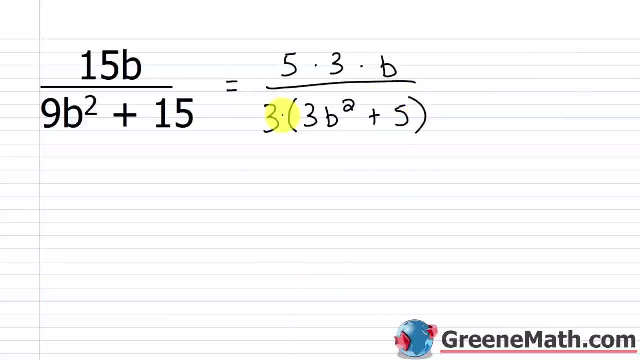 Now, I'm going to cancel a common factor of 3 only. Why? This is multiplication. So I have a factor. 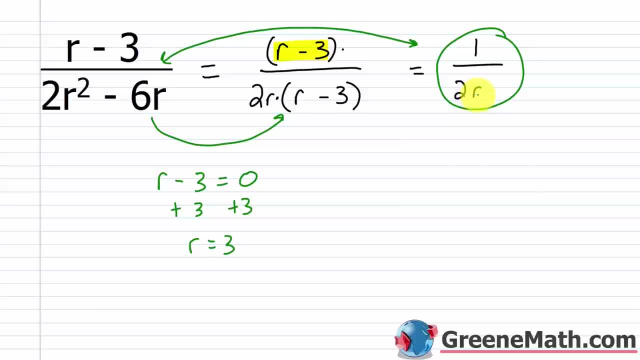 over two r. I can plug in a three right. So two times three is six. I'd have one over six. So that's where students get confused. So you almost need like a side note there to kind of explain that and say well, 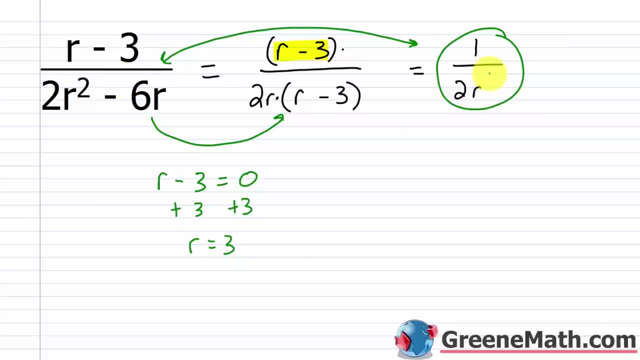 they are equal, but not if r is equal to three. And the way you say that is, you look at your original rational expression and you look at that denominator to give you your proper restricted values. okay, So if you stick with the original denominator, you're always going to be good to go. 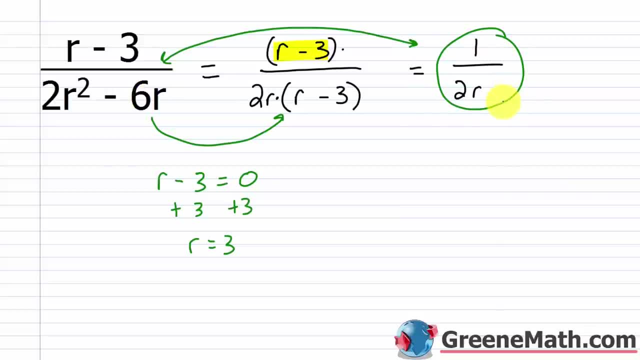 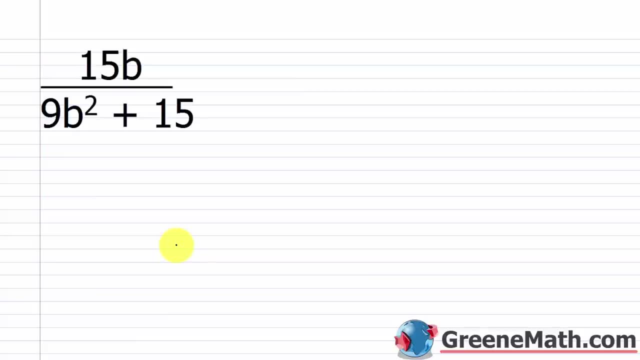 You don't want to look at the simplified one because you might not list all of them. All right, let's take a look at it all. So we have 15b over 9b squared plus 15.. So what can I do here? Again, I want to factor the numerator. 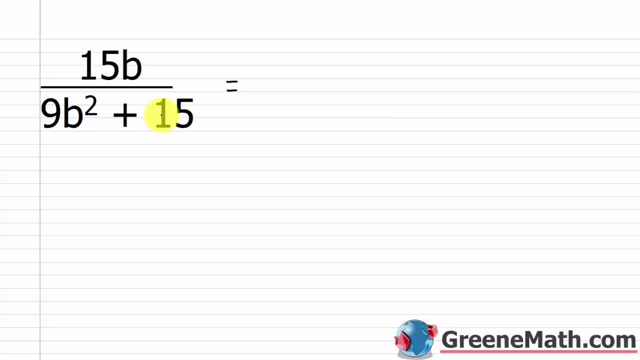 denominator And for the numerator, I know I can break 15 into five times three. so let's go ahead and just do that five times three, And then I have that b. so times b In the denominator, I have 9b squared plus 15.. So what's? 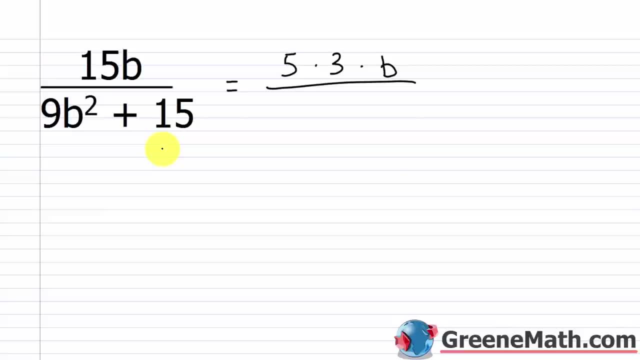 common to each term. there would be a three right. So if I pulled a three out I would have what I'd have: three b squared plus five. Now I'm going to cancel each line to the other side. I'm going cancel a common factor of three only Why This is multiplication. So I have a factor. 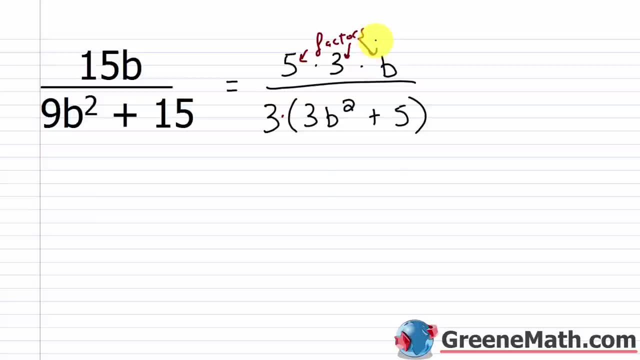 Let me just write factors here and point to all of them, And then this is a factor and this is a factor. So what can I cancel? I can cancel common factors, So I can cancel this three with this three. Okay, So once I've done that, the simplified numerator is five B and the simplified denominator 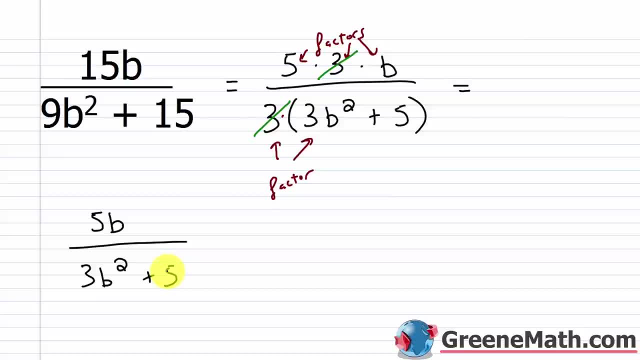 is three B squared plus five. That's all I can do. Don't make the mistake again. like most students do, They go. okay, I can cancel this B with this and that's a one, And then I can cancel, you know. 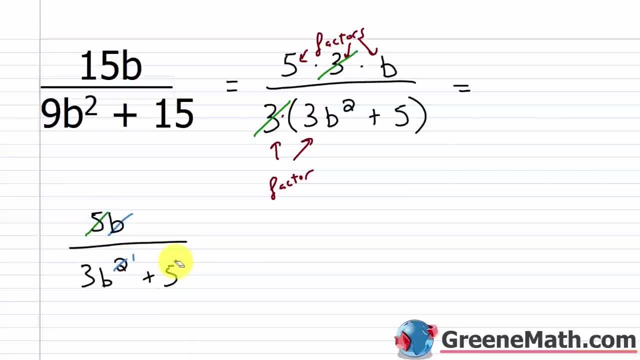 oh, look, there's a five here that I can cancel this with this. You can't. You're out of common factors to cancel Again. it's got to be a factor, a common factor between the numerator and denominator. This three is a factor. This three is a factor. It's multiplying this three, B squared. 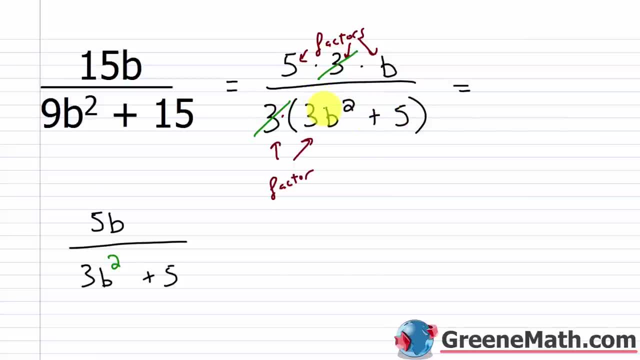 plus five. So I can cancel this three with this three, And then I can cancel this three with this five. Again, very common mistake, And I want you just to understand that moving forward. So your simplified answer here is: five B over three B squared plus five. All right, let's take a look. 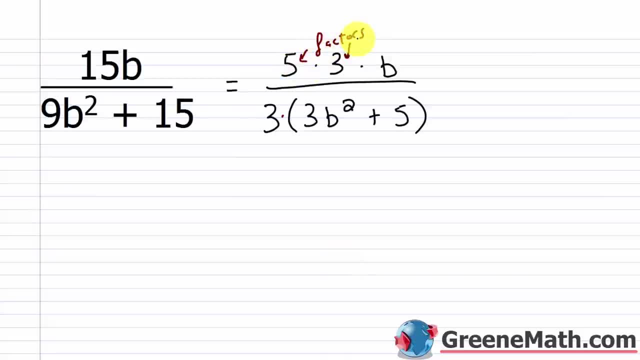 Let me just write factors here, and point to all of them. And then this is a factor, and this is a factor. So what can I cancel? I can cancel common factors. So I can cancel this 3 with this 3, okay? So once I've done that, the simplified numerator is 5b, and the simplified denominator is 3b squared plus 5. That's all I can do. 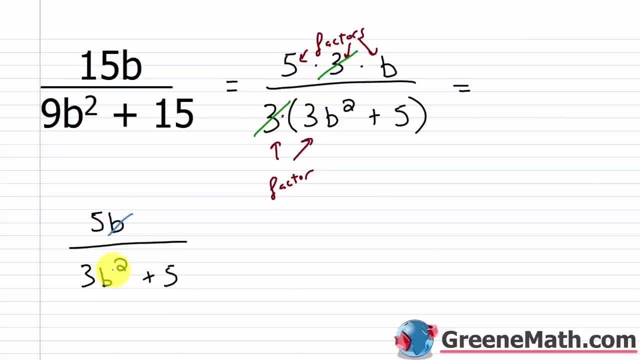 Don't make the mistake, again, like most students do, they go, okay, I can cancel this b with this, and that's a 1, and I can cancel, you know, oh look, there's a 5 here, and I can cancel this with this. You can't. You're out of common factors to cancel. Again, it's got to be a factor, a common factor between the numerator and denominator. This 3 is a factor, this 3 is a factor, it's multiplying this 3b squared plus 5. Again, very common mistake, and I want you just to understand that moving forward. 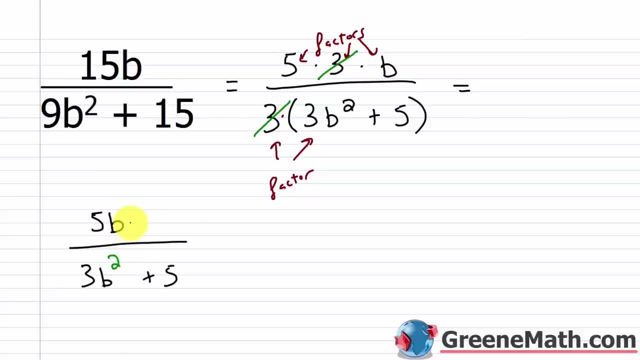 So your simplified answer here is 5b over 3b squared plus 5. All right, let's take a look at another one. 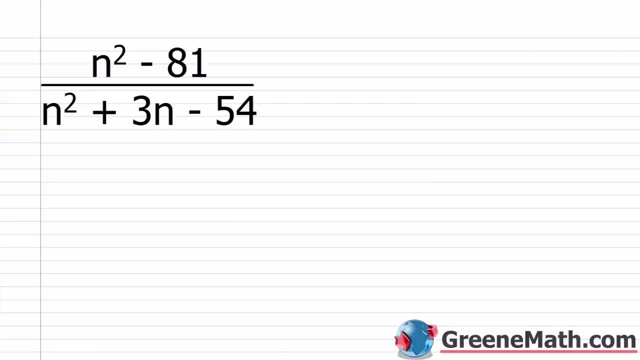 We have n squared minus 81 over n squared plus 3n minus 54. So if I factor the numerator... I notice that is the difference of two squares. This is n plus 9 times n minus 9. These are being multiplied together, so each is a factor. This is over n squared plus 3n minus 54. So let's go ahead and set up our parentheses here, put an n here and an n here. 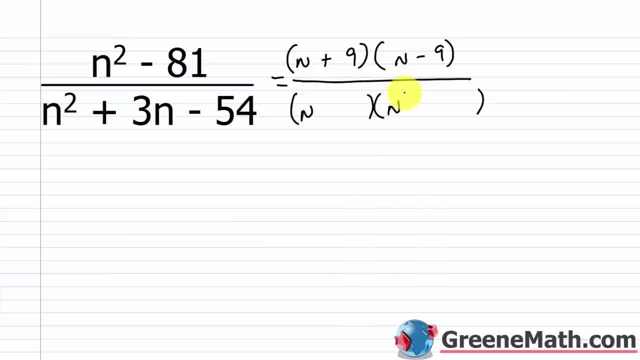 And a typical kind of trick to speed yourself up, if you get stuff like this on a test, you know they're going to give you stuff that cancels 99% of the time. So you're going to have to do this. You're going to have to do this 99% of the time. So it's probably going to be that one of these is going to be a 9. It could be plus 9 or minus 9. They make it to where one of them is going to cancel. So if I look at this real quick, I see that I need two integers that sum to 3 and multiply to negative 54. 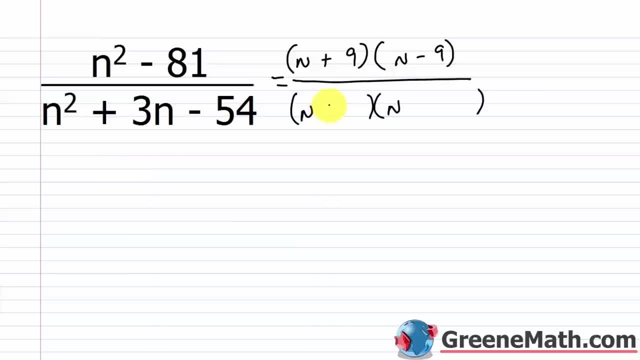 So if I think about that, I can do positive 9, so n plus 9, and then negative 6. 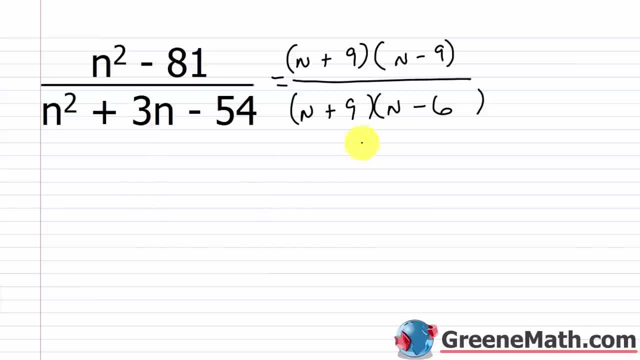 The sum is going to be positive 3. The product is going to be negative 54. And then I see that... 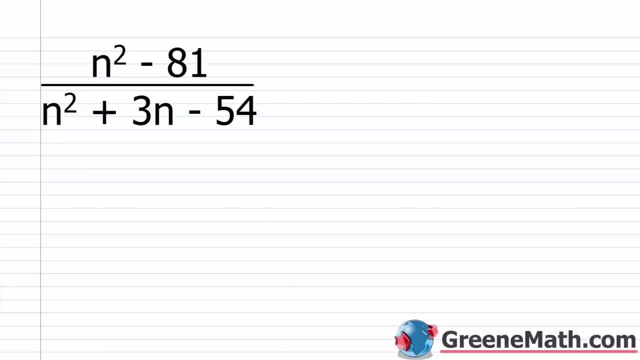 at another one, We have N squared minus 81 over N squared plus three, N minus 54.. So if I factored the numerator I noticed that is the difference of two squares. This is N plus nine times N minus nine. These are being multiplied. 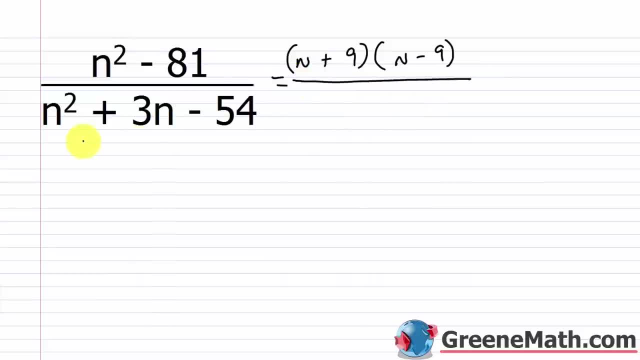 So each is a factor. This is over N squared plus three, N minus 54.. So let's go ahead and set up our parentheses here, put an N here and an N here, And a typical kind of trick to speed yourself up. If you get stuff like this on a test, you know they're going to give you stuff that cancels. 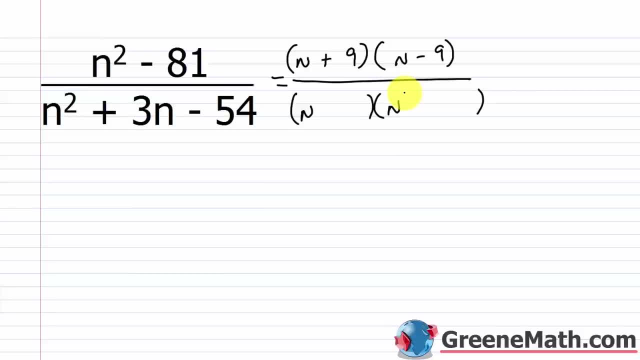 99% of the time. So it's probably going to be that one of these is going to be a nine. It could be plus nine or minus nine. They make it to where one of them is going to cancel. So if I look at this, 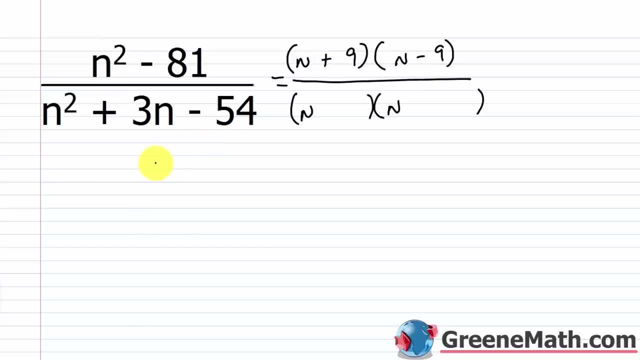 real quick, I can see that it's going to be a nine. So if I look at this real quick, I can see that I need two integers that sum to three and multiply to negative 54. So if I think about that, I can do. 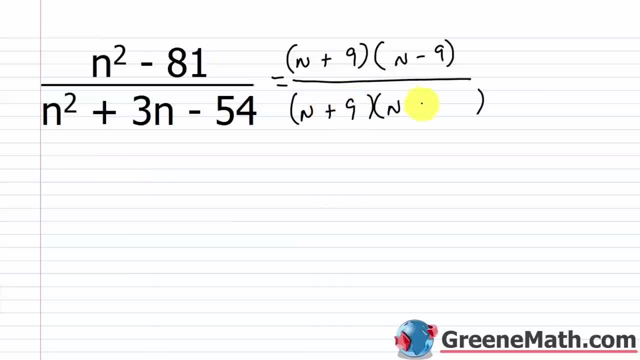 positive nine, So N plus nine, and then negative six, The sum is going to be positive three. The product is going to be negative 54. And then I see that this would cancel with this right. Again, these are factors. Those factors are canceling, And so what I'm left with is N minus nine. 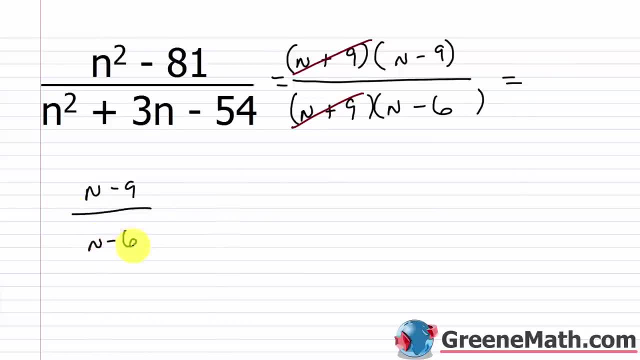 over N minus 54.. Let's take a look at another one. So we have X squared minus 11, X plus 18 over X squared minus four. So we notice right away the bottom is what the difference of two squares This is X. 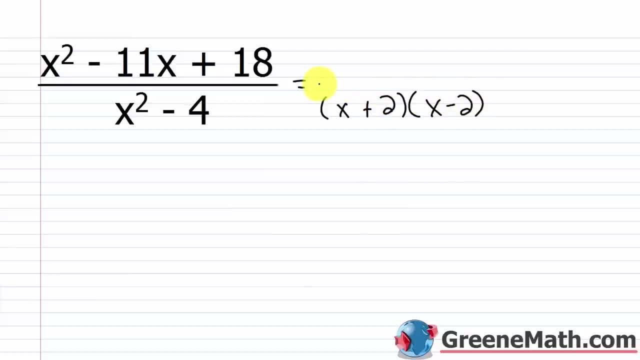 plus two times X, minus two on the top, Go ahead and set this up. So again, kind of a trick is to realize that it's going to probably be a plus two or minus two in one of those scenarios, because they make these things to where? 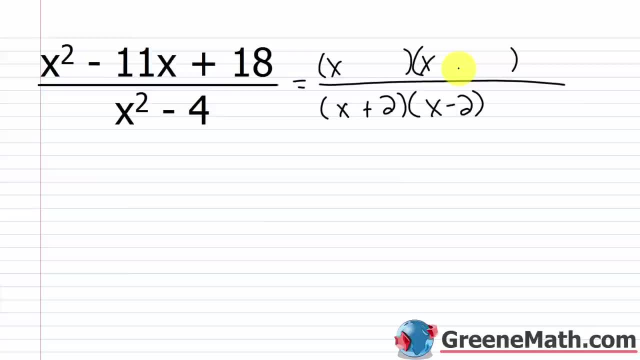 something's going to cancel 99% of the time. You get some problems where it doesn't, but most of the time it does. So I need two integers whose sum is negative 11 and whose product is 18.. So I know that's going to be negative two, negative two and negative nine. Negative nine plus negative two is 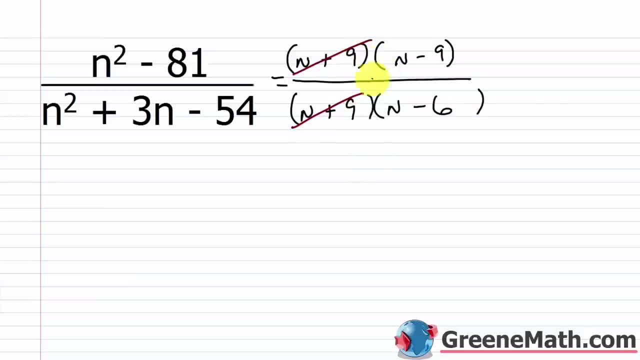 This would cancel with this. Right? Again, these are factors. Those factors are canceling. And so what I'm left with is n minus 9 over n minus 6. Let's take a look at another one. 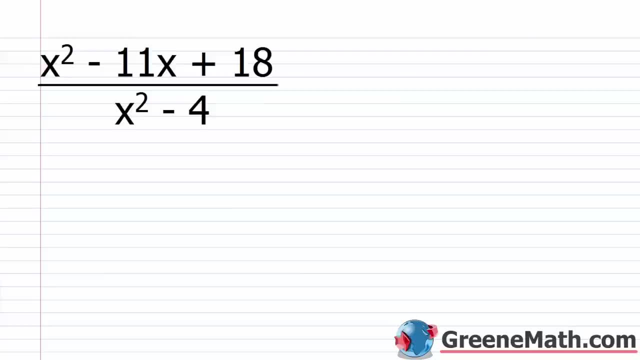 So we have x squared minus 11x plus 18 over x squared minus 4. So we notice right away the bottom is what? The difference of two squares. This is x plus 2 times x minus 2. On the top... Go ahead. Go ahead and set this up. So again, kind of a trick is to realize that it's going to probably be a plus 2 or a minus 2 in one of those scenarios because they make these things to where something's going to cancel. 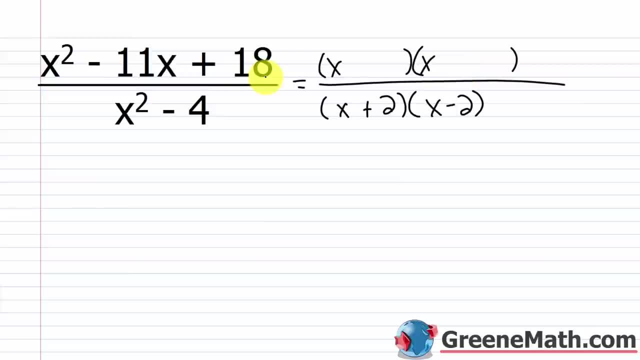 99% of the time. You get some problems where it doesn't, but most of the time it does. 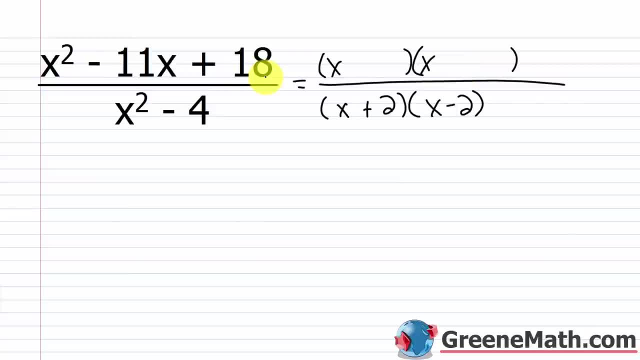 So I need two integers whose sum is negative 11 and whose product is 18. So I know that's going to be negative 2, negative 2, and negative 9. Negative 9 plus negative 2 is negative 11. Negative 9 times 2. Times negative 2 is positive 18. So I can cancel common factors here. Cancel this factor of x minus 2 with this factor of x minus 2, and what I'm left with is x minus 9 over x plus 2. 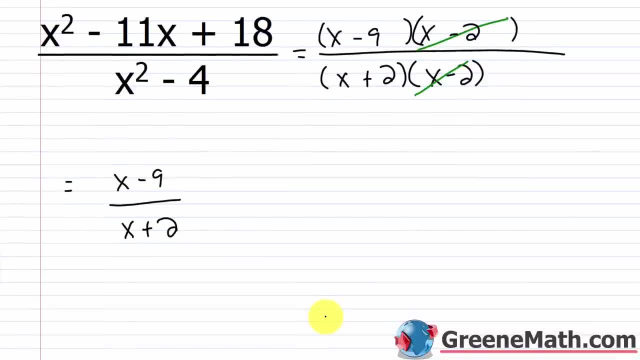 Let me just show you why it's useful to simplify these things. Let's say I said that would I rather evaluate when it looks like this or when it looks like this? 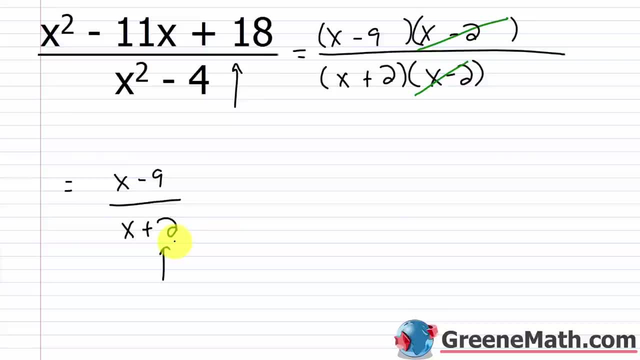 Let's say I said x is equal to 5. Give me the value for the rational expression. Well here I can say 5 minus 9 is negative 4 over 5 plus 2. That's 7. So I get negative 4 sevenths. Nice and easy. 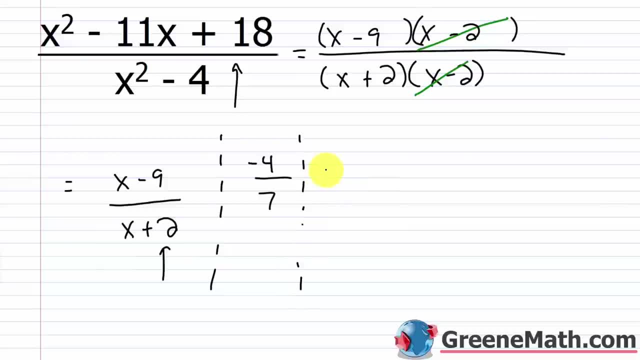 Very quick. If I did it up here, I would have 5 squared. That's 25. Minus 11 times 5. That's 7. Minus 5. That's 55. Plus 18. You think about how much more work this is. 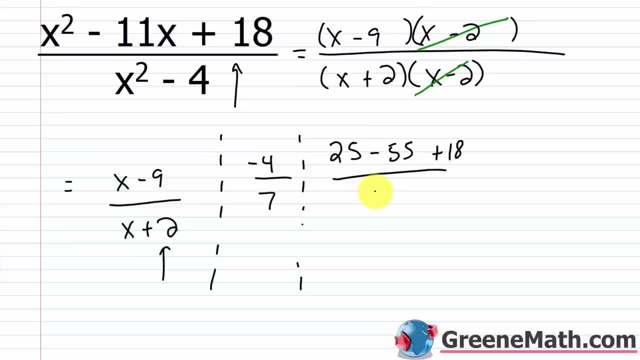 And then over, 5 squared is 25. 25 minus 4 is 21. So let's do this. 25 minus 55 is negative 30. Negative 30 plus 18 is negative 12. So this would be negative 12 over 21. Then I've got to simplify this. Both are divisible by 3. 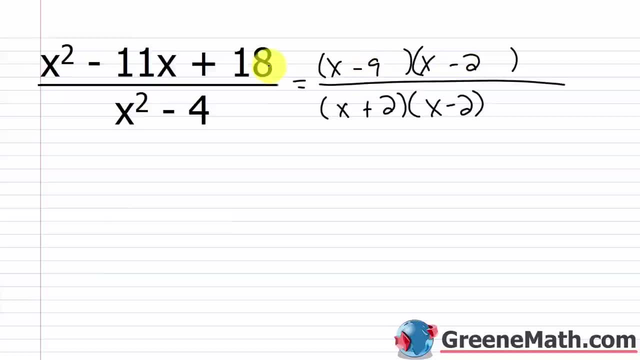 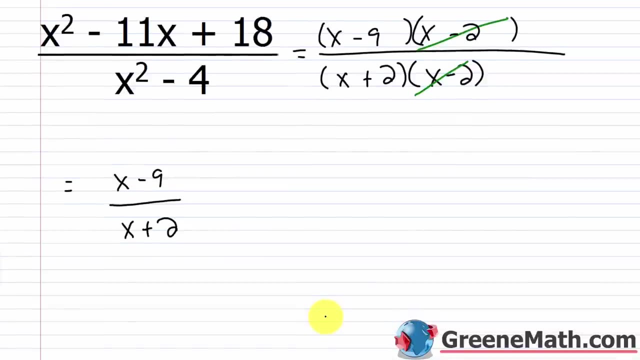 negative 11. Negative nine times negative two is positive 18. So I can cancel common factors here. cancel this factor of X minus two with this factor of X minus two, And what I'm left with is X minus two over X plus two. Let me just show you why it's useful to simplify these things. Let's say I said that 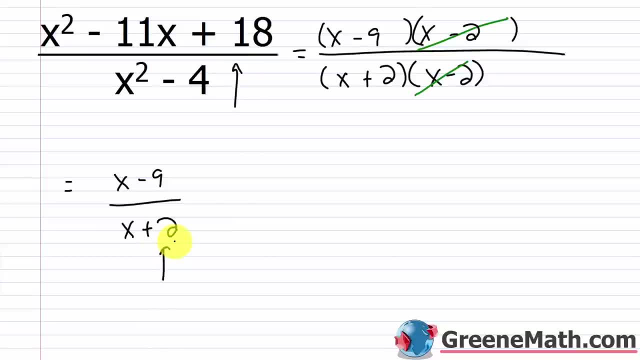 would I rather evaluate when it looks like this or when it looks like this. Let's say I said X is equal to five. Give me the value for the rational expression. Well, here I can say: five minus nine is negative four over five plus two that's seven. So I get negative four. sevenths. nice and easy, very quick. 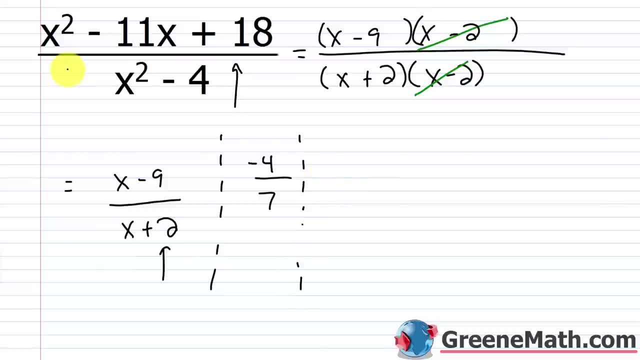 If I did it up here, I would have: five squared, that's 25.. Minus 11 times five, that's 55, plus 18.. You think about how much more work this is. And then over five squared is 25,. 25 minus four is 21.. So let's do this: 25 minus 55 is negative 30.. 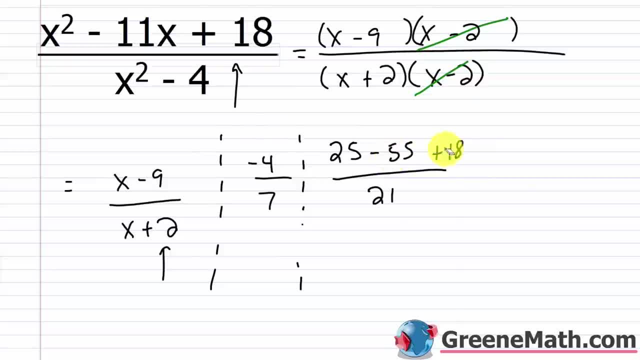 Negative 30 plus 18 is negative 12.. So this would be negative 12 over 21.. Then I've got to simplify this. both are divisible by three, So this would be negative four and this would be seven. So you get the same answer either way. 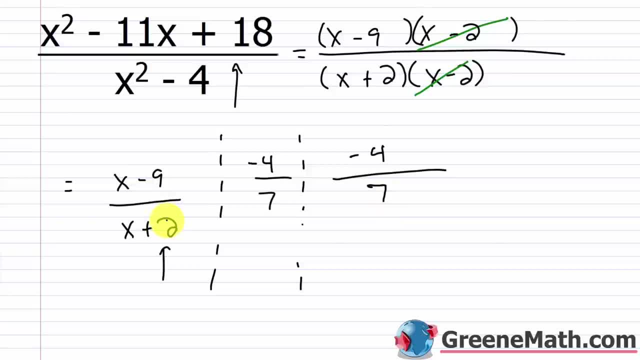 but look how much longer it took. So that's one reason why we go through the process: to simplify these things. It makes it easier if you need to plug in a value for your variable and see what that rational expression is equal to. All right, let's take a look at one final problem. 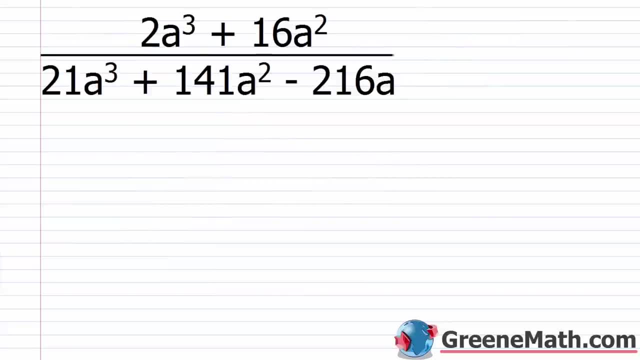 So we have two A cubed plus 16 A squared over 21 A cubed plus 141 A squared minus 216 A 216a. So in the numerator I can factor out a 2a squared and that's going to give me an a plus. 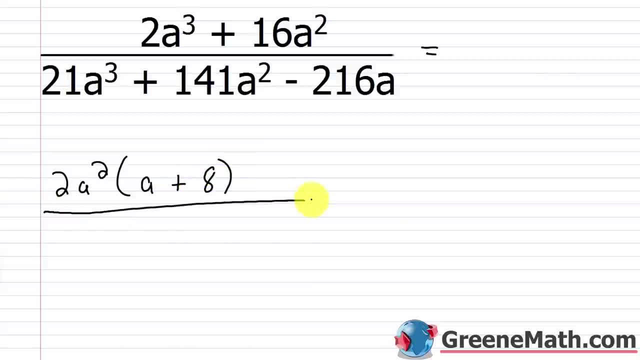 8. In the denominator I can see right away that I can pull out an a, but everything is also divisible by 3. So I can pull out a 3a, So I'd have 3a times, you'd have 7a squared plus 47a. So this would be negative 4. And this would be 7. So you get the same answer. 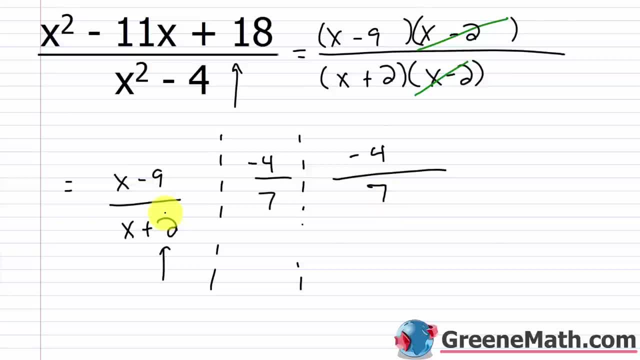 Either way. But look how much longer it took. So that's one reason why we go through the process to simplify these things. 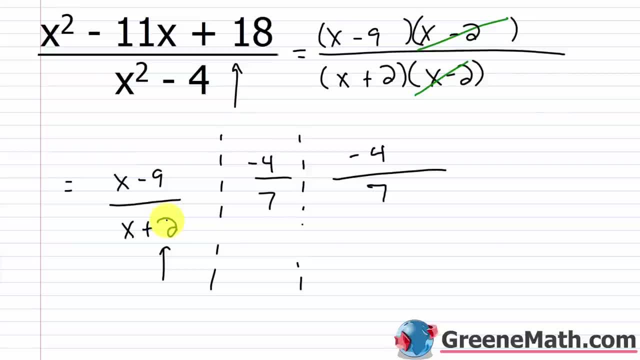 It makes it easier if you need to plug in a value for your variable and see what that rational expression is equal to. All right. Let's take a look at one final problem. 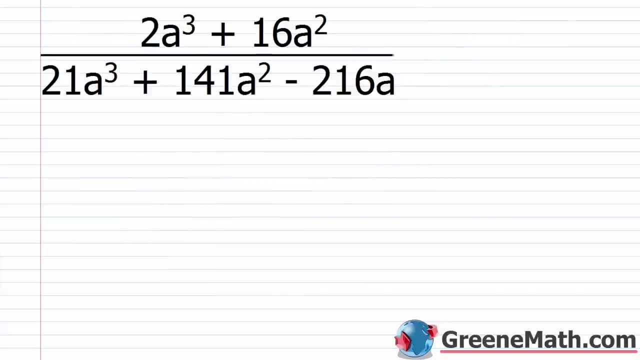 So we have 2a cubed plus 16a squared over 21a cubed plus 141a squared minus 216a. So in the numerator, I can factor out a 2a squared. 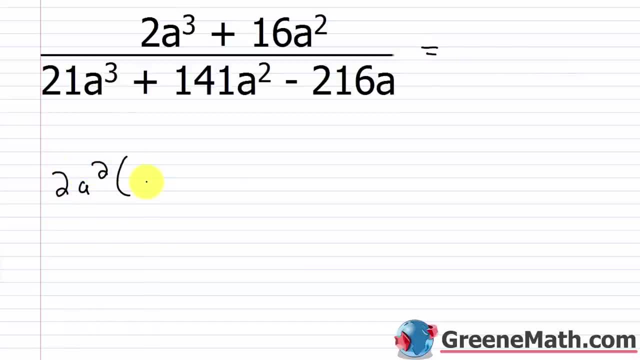 And that's going to give me an a plus 8. In the denominator, I can see right away that I can pull out an a. But everything is also divisible by 3. So I can pull out a 3a. 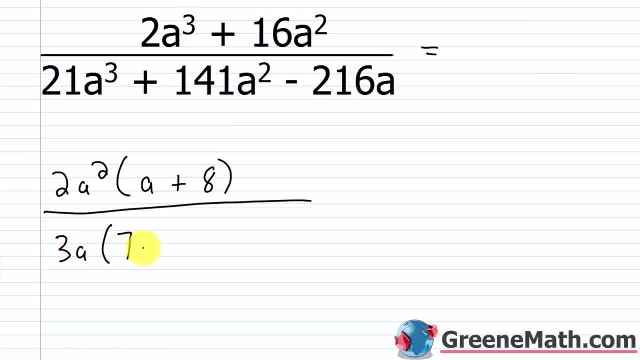 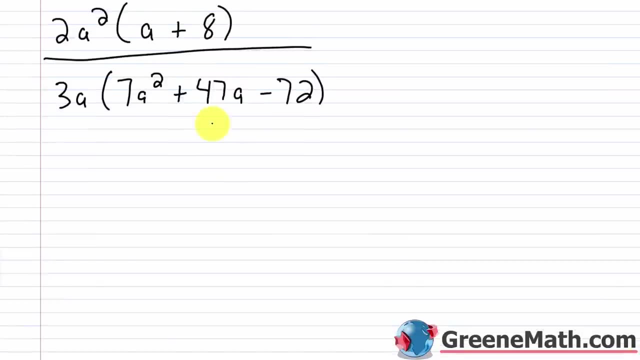 So I'd have 3a times, you'd have 7a squared plus 47a, then minus 72. So for the denominator, let's factor this down here real quick. I'm going to use the grouping method. 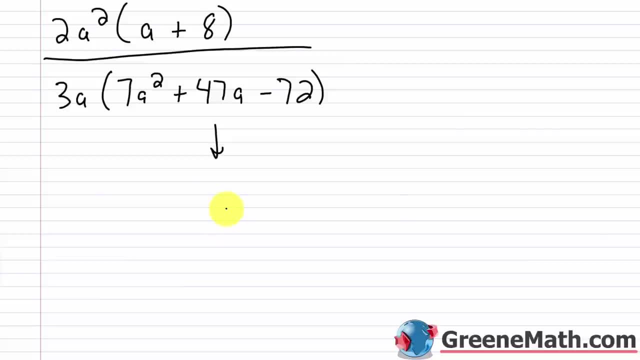 Give me two integers whose product is 7 times negative 72, which would be negative 504, and whose sum is 47. 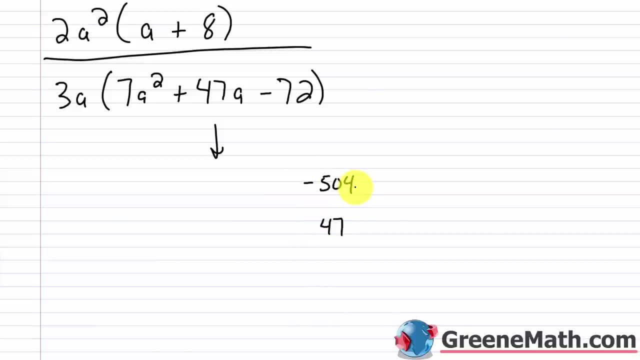 So for this one, because I don't know the factors of 504 off the top of my head, I'd have to make a factor tree. So 504. I know I could start out with divisibility by 4. So I could do 4 times 126. 4 is 2 times 2. All right. 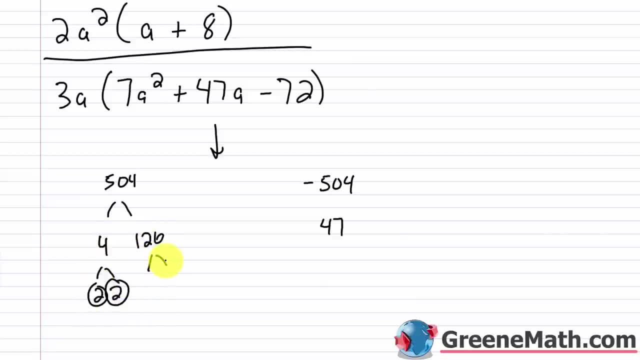 I'm going to do 2 times 2. For 126, I could do 2 times 63. 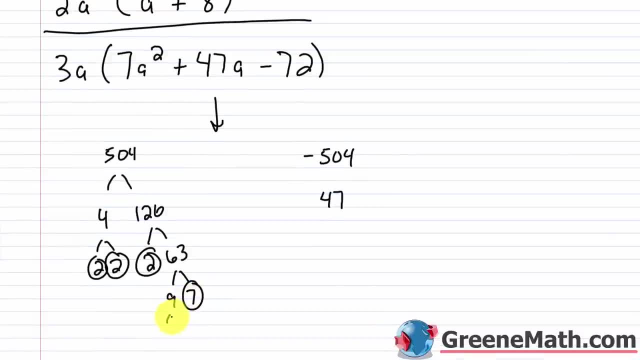 So 2 is prime. 63 is 9 times 7. 7 is prime. And 9 is 3 times 3. And those are prime. 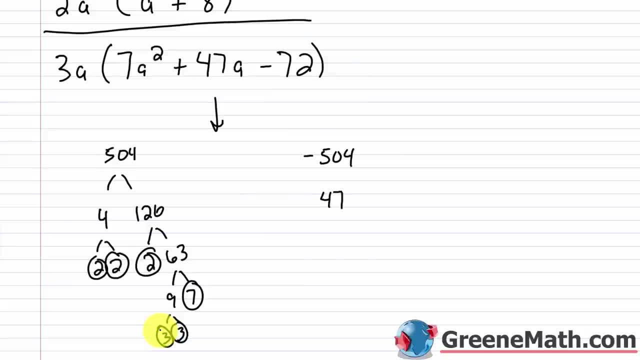 So I'm looking for a sum of 47. So let me think about this. 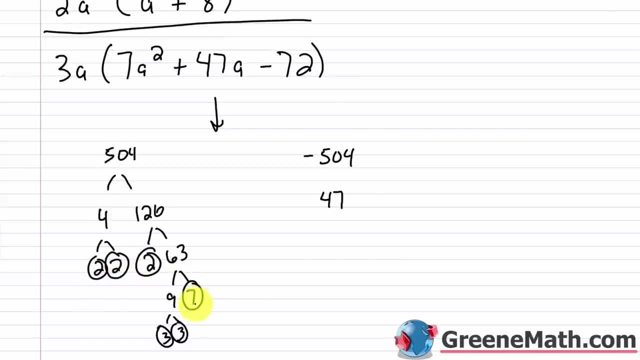 I can do 2 times 2 times 2, which is 8, times 7, which is 56 times 9. So 56 times 9 would give me 504. 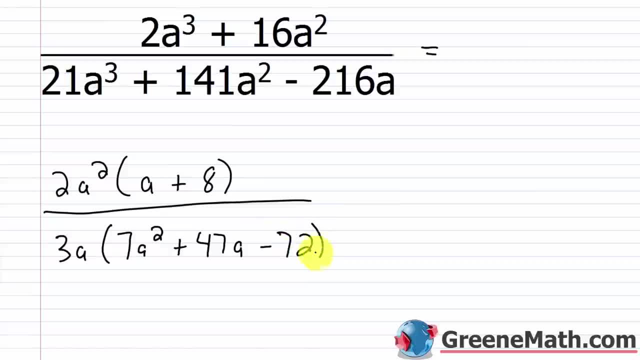 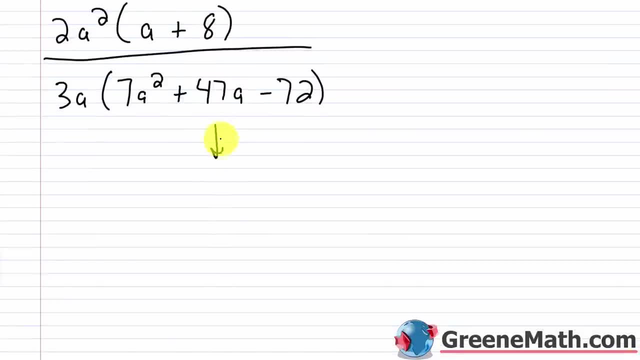 then minus 72.. So for the denominator, let's factor this down here real quick. I'm going to use the grouping method. Give me two integers whose product is 7 times negative 72, which would be negative 504, and whose sum is 47. So for this one, because I don't know the factors, 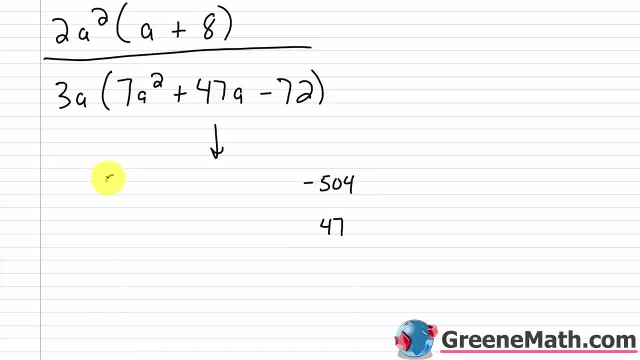 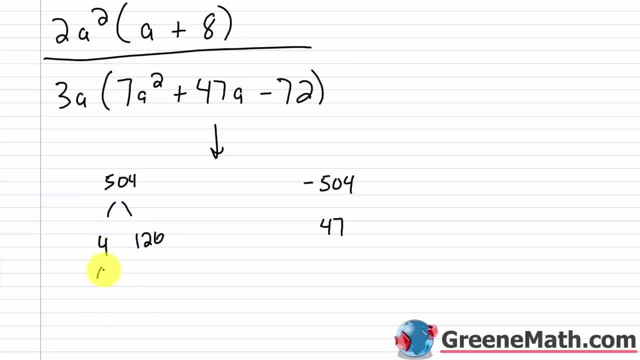 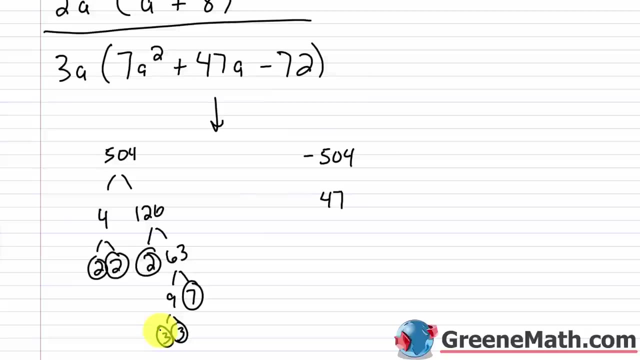 by 4, so I could do 4 times 126. 4 is 2 times 2 for 126. I could do 2 times 63. so 2 is prime, 63 is 9 times 7, 7 is prime and 9 is 3 times 3, and those are prime. so I'm looking for a sum of 47. so let 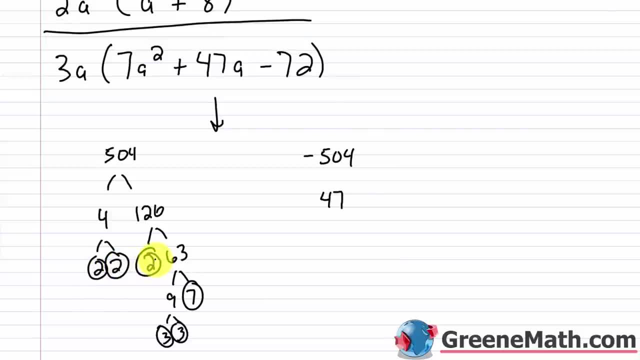 me think about this. I can do 2 times 2 times 2, which is 8 times 7, which is 56 times 9. so 56 times 9 would give me 504, and then if I did positive 56 and negative 9, that would give me. 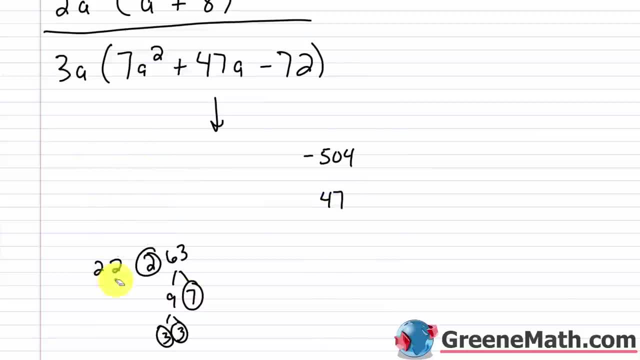 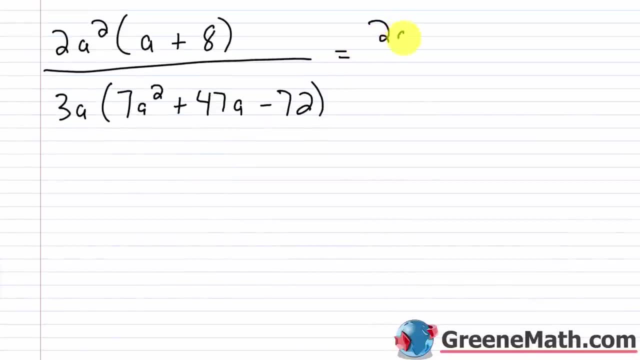 47 as a sum. so let's go ahead and do that, let's erase all this, and so I'll put this as equal to: we'll have 2a squared and times a plus 8 over, we'll have 3a times. let me kind of factor this: 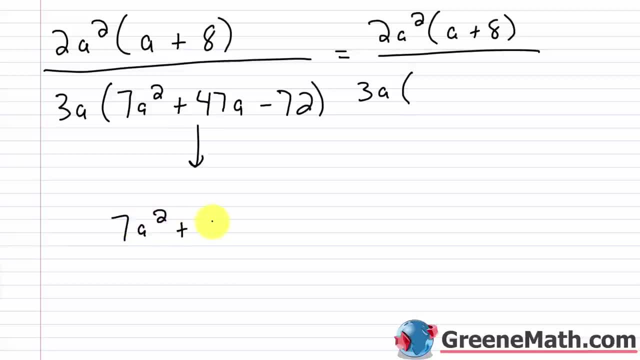 down here. so so 7a squared plus. I'm going to put positive 56a and then negative 9a and minus 72. if I factored this guy, I'd pull out a 7a from the first group and I'd have a plus 8. 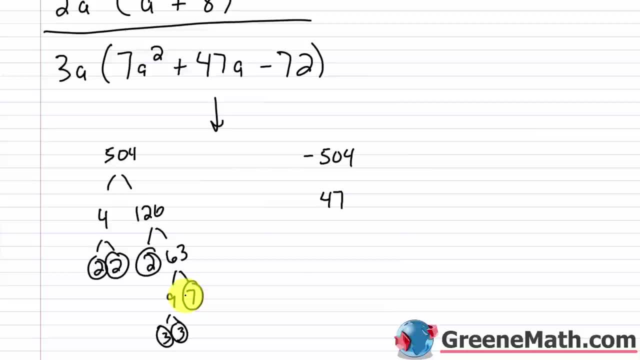 And then... So if I did positive 56 and negative 9, that would give me 47 as a sum. So let's go ahead and do that. Let's erase all this. 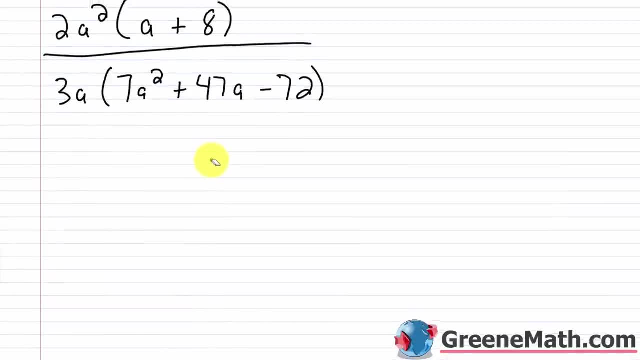 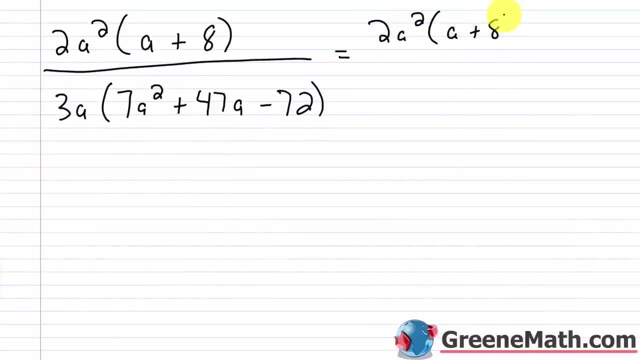 And so I'll put this as equal to... We'll have 2a squared and times a plus 8 over... We'll have 3a times... 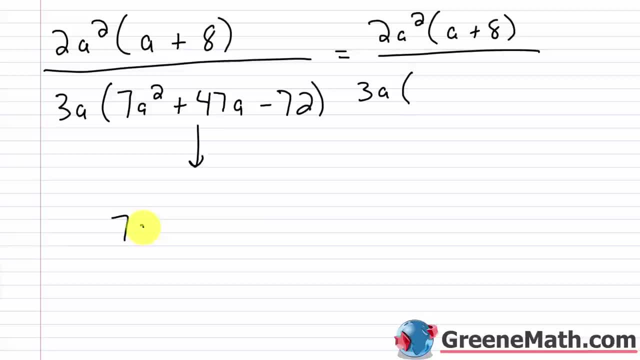 Let me kind of factor this down here. So 7a squared plus... I'm going to put... Positive 56a and then negative 9a and minus 72. If I factored this guy, I'd pull out a 7a from the first group and I'd have a plus 8. From the second guy, I'd pull out a negative 9 and I'd have a plus 8. So this is going to be 7a minus 9 times a plus 8. So then I can easily see what I can cancel here. Cancel this with this, right? Common factor of a plus 8. 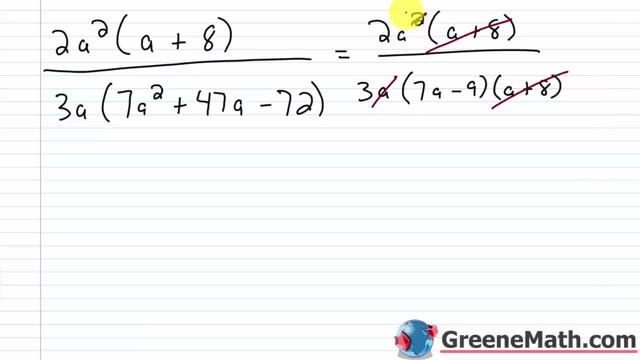 And I can also cancel this a with one factor of a up here. So what I'm going to be left with is a 2a in my numerator over 3 times we have 7a minus 9. 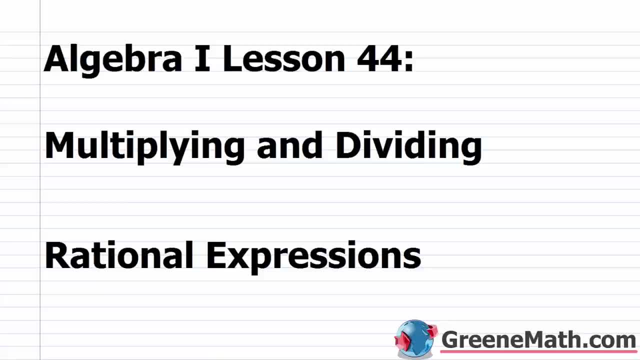 Hello and welcome to Algebra 1, Lesson 44. 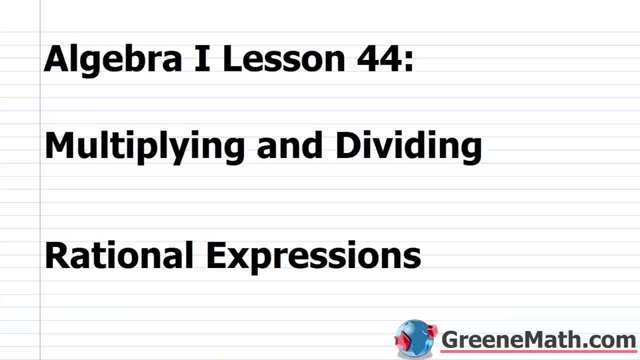 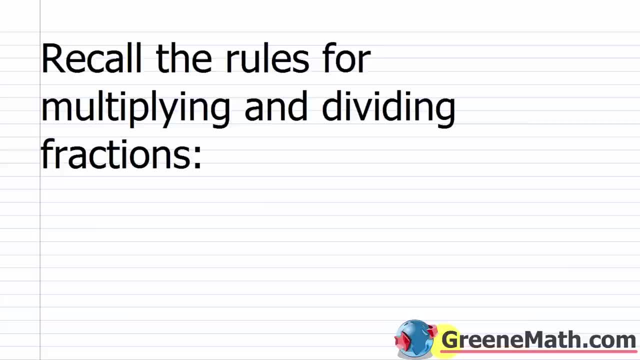 In this video, we're going to learn about multiplying and dividing rational expressions. So in our last lesson, we started talking about rational expressions. We learned how to simplify rational expressions and we learned how to find the restricted values for a rational expression. Now we're going to move on and start talking about some operations with rational expressions. 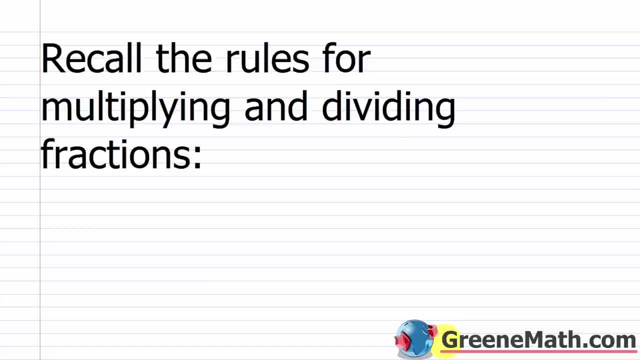 And kind of the easiest ones to start with would be multiplication and division. 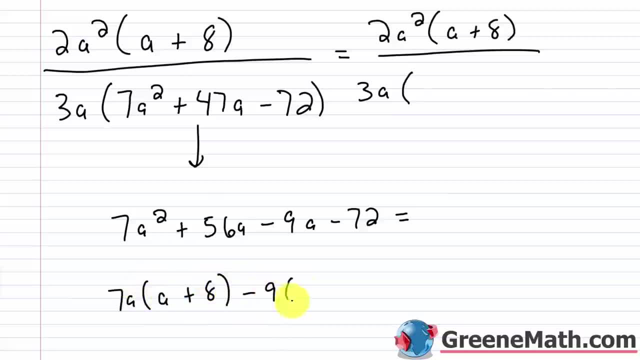 from the second guy. pull out a negative 9 and I'd have a plus 8. so this is going to be 7a minus 9 times a plus 8. so then I can easily see what I can cancel here. cancel this with this right common factor of a. 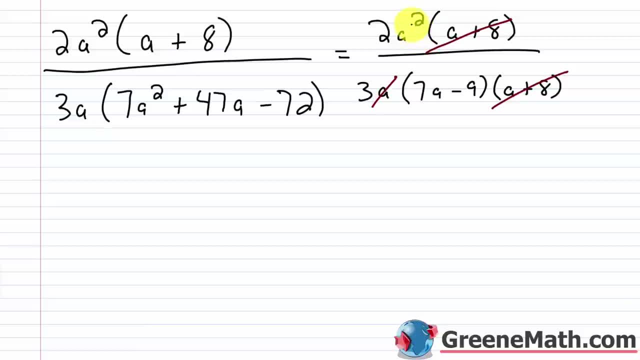 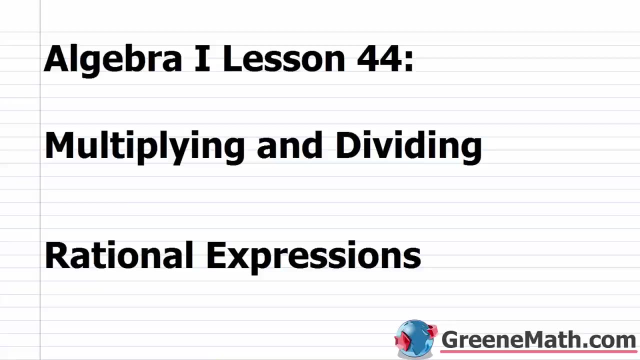 plus 8, and I can also cancel this a with one factor a up here. so what I'm going to be left with is a 2a in my numerator. over 3 times, we have 7a minus 9. hello and welcome to algebra 1. 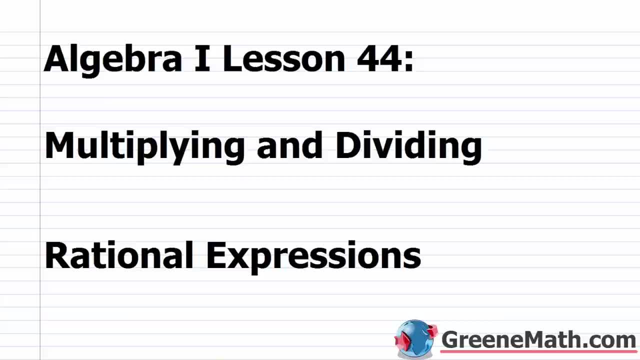 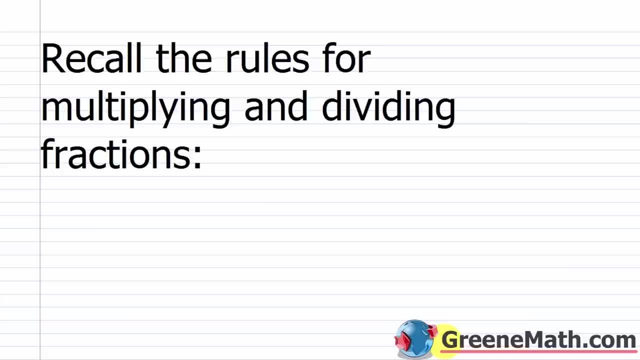 lesson 44. in this video we're going to learn about multiplying and dividing rational expressions. so in our last lesson we started talking about rational expressions. we learned how to simplify rational expressions and we learned how to find the restricted values for a rational expression. now we're going to move on and start talking about some operations with rational expressions. 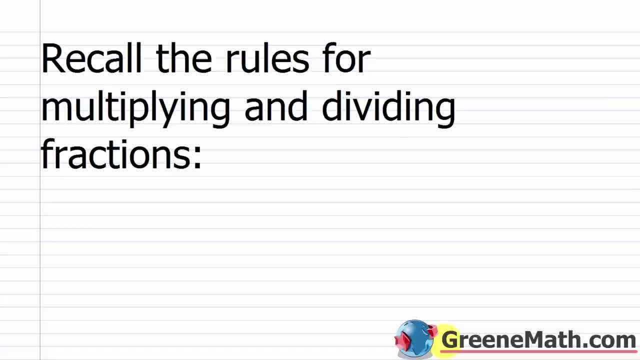 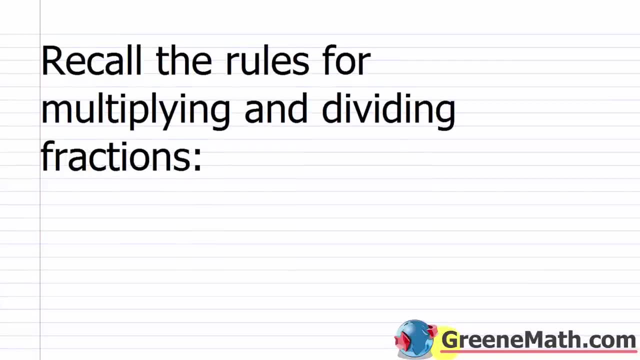 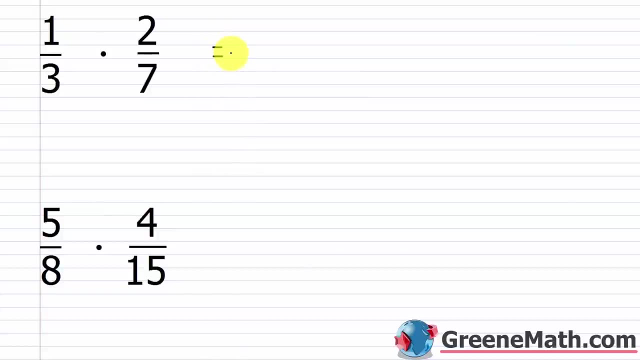 and kind of the easiest ones to start with would be multiplication and division. now, if you know how to multiply and divide fractions, the process is very, very similar. so let's start by looking at 1, 3rd times, 2, 7ths. so what we want to do here is we want to multiply the numerator times the numerator. 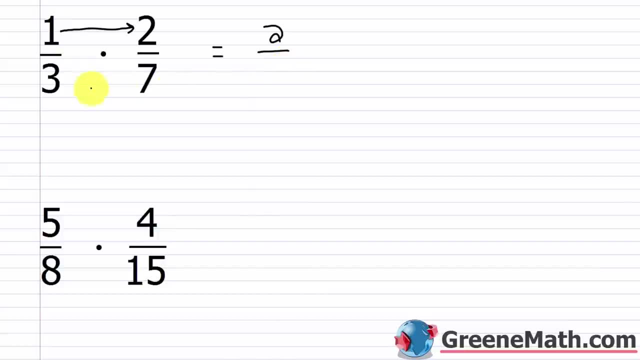 so 1 times 2 is 2. we want to place this over the denominator times the denominator. so 3 times 7 is 21. so you get 2 over 21 there. now remember: when you're working with fractions, you want the fraction to be simplified or, as they say, reduced to its lowest terms. now you can look at 2 and you can. 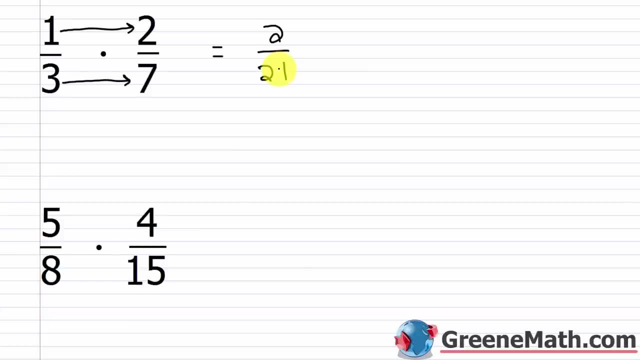 look at 21 and you can tell that there's nothing that's going to be reduced to its lowest terms. and you can kind of start from over here. remember, we're allowed to cross cancel. if I look at 1 and I look at 3, there's nothing in common there other than 1. if I look at 2 and I look at 7, nothing in. 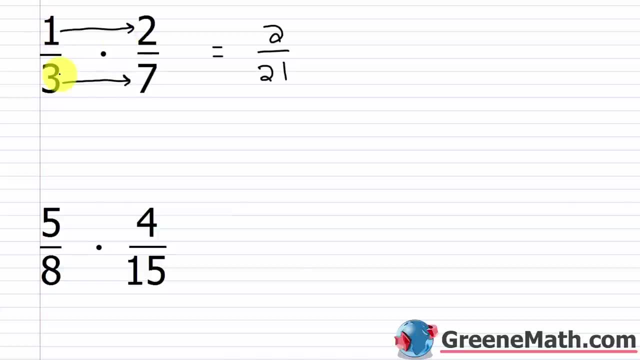 common other than 1. and then I can look crossways: 1 and 7, 2 and 3: nothing in common there other than 1. so we would say that 2 over 21 is simplified or again reduced to its lowest terms. now let's. 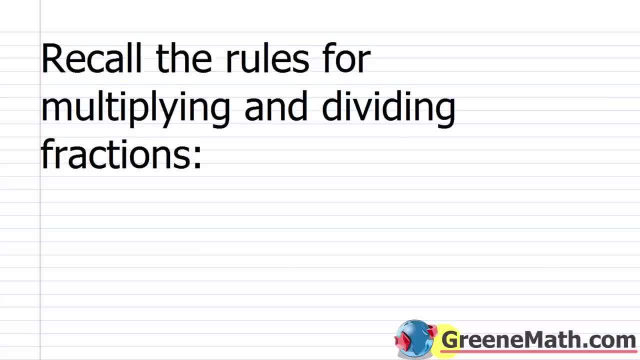 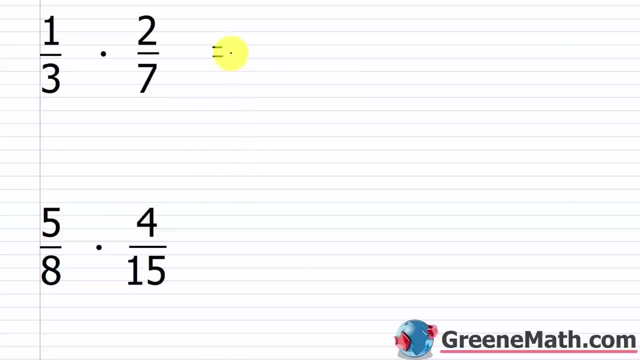 Now if you know how to multiply and divide fractions, the process is very, very similar. So let's start out by looking at 1 third times 2 sevenths. So what we want to do here... So we want to multiply the numerator times the numerator. So 1 times 2 is 2. And we want to place this over the denominator times the denominator. So 3 times 7 is 21. So you get 2 over 21 there. 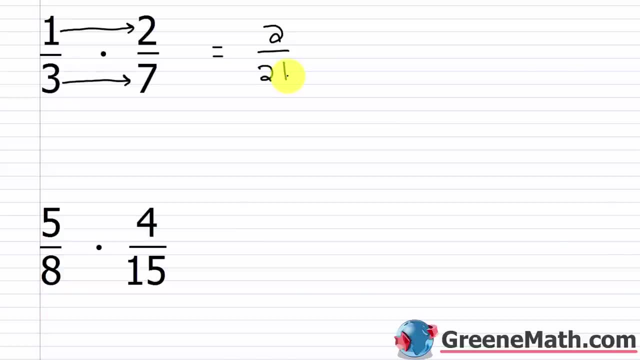 Now remember, when you're working with fractions, you want the fraction to be simplified or 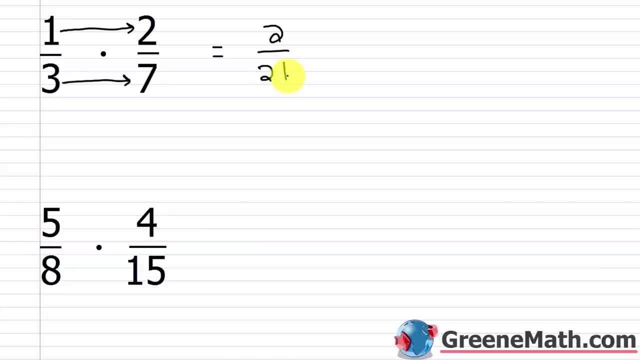 as they say, reduced to its lowest terms. Now you can look at 2 and you can look at 21 and you can tell that there's nothing that's going to be common other than 1. And you can kind of start from over here. Remember, we're allowed to cross-cancel. If I look at 1 and I look at 3, there's nothing in common there other than 1. If I look at 2 and I look at 7, nothing in common other than 1. And then I can look crossways, 1 and 7, 2 and 3, nothing in common there other than 1. 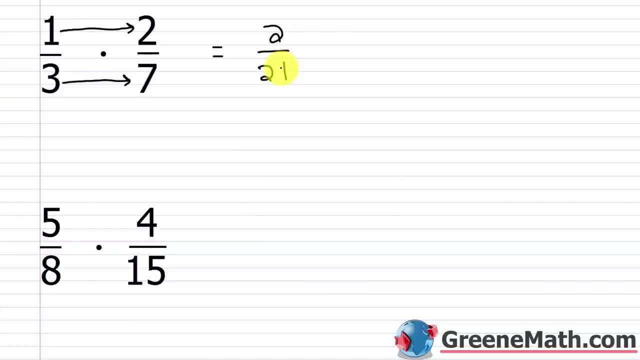 So we would say that 2 over 21 is simplified, or again, reduced to its lowest terms. 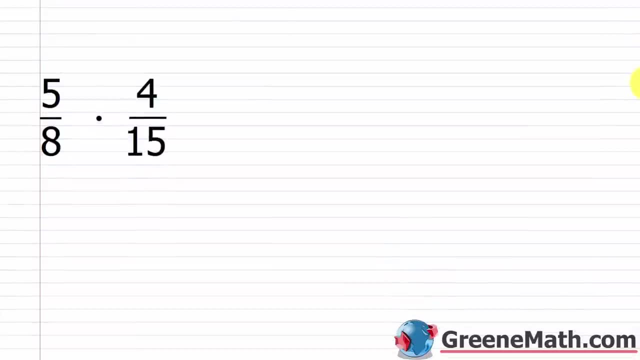 Now let's take a look at one where you can do some simplification. We have 5 eighths times 4 fifteenths. So what I can do... 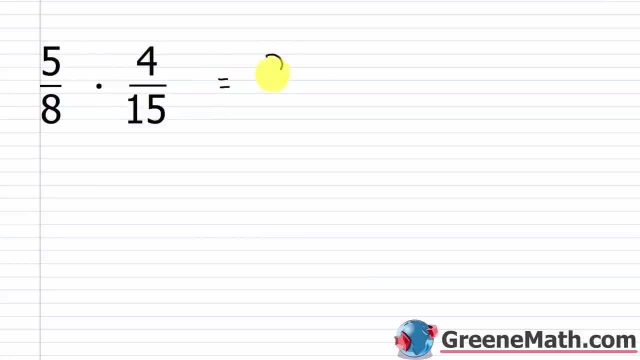 I can multiply everything together first, 5 times 4 is 20, over 8 times 15, which is 120. 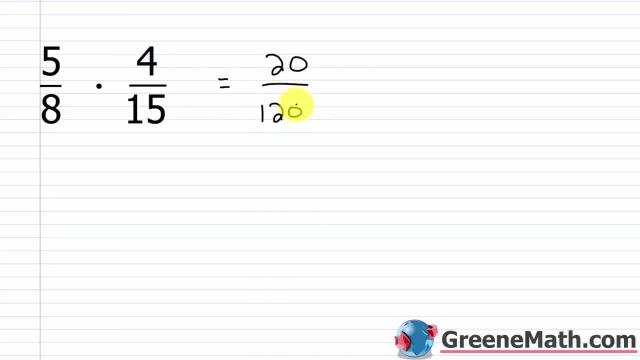 But then I have to go through and simplify, so that doesn't make much sense. So for most people, what they'll do is they will cross-cancel or cancel before they even start the multiplication process. 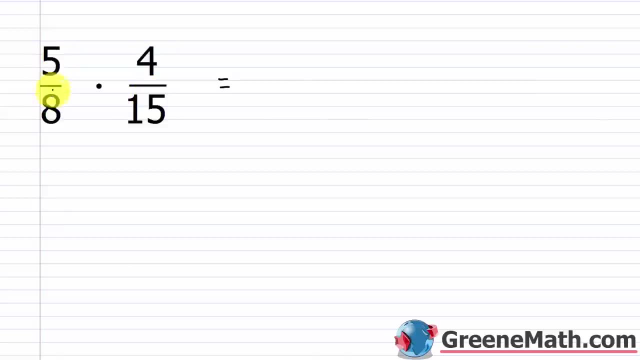 So you look between numerator and denominator of each fraction first. Look between 5 and 8, there's nothing you can cancel, 4 and 15, nothing to cancel. Then I would look crossways. So I would look between 5 and 15. 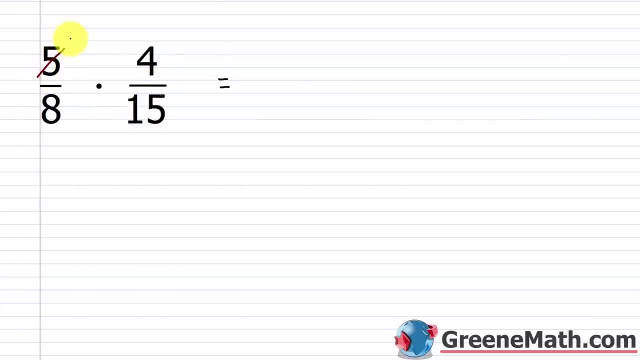 There's a common factor of 5, so 5 divided by 5 is 1, 15 divided by 5 is 3. And I'd look crossways again. Between 8 and 4, there's a common factor of 4. So divide this by 4, I get 1. Divide this by 4, I get 2. 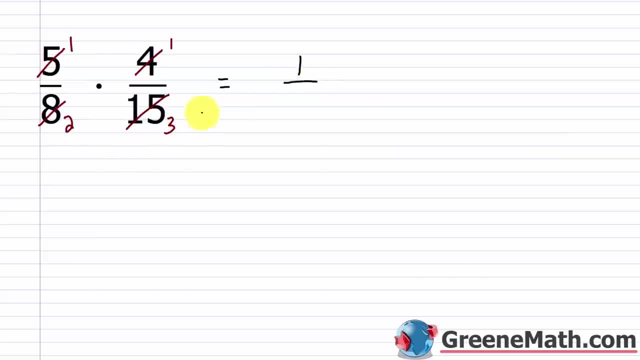 So now if I multiply, 1 times 1 is 1, over 2 times 3, that's 6. 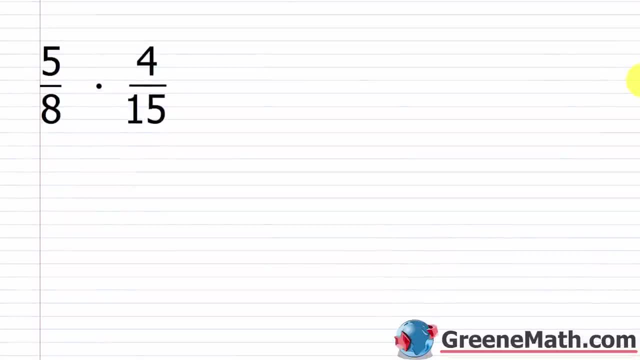 take a look at one where you can do some simplification. we have 5 eighths times 4- 15ths. so what I can do is I can multiply everything together first: 5 times 4 is 20 over 8 times 15, which is 120. but then I have to go through and simplify so that doesn't make. 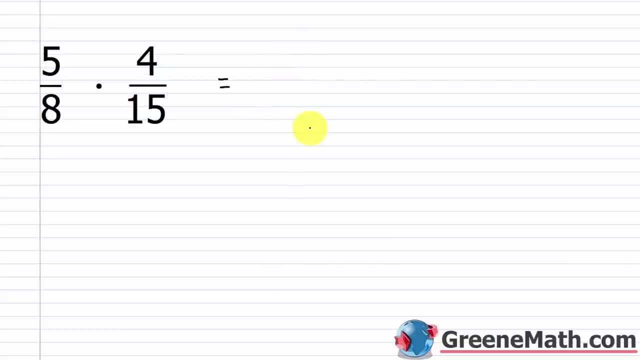 much sense. so for most people what they'll do is they will cross cancel or cancel before they even start the multiplication process. so you look between numerator and denominator of each fraction. first look between 5 and 8: there's nothing you can cancel. 4 and 15: nothing to. 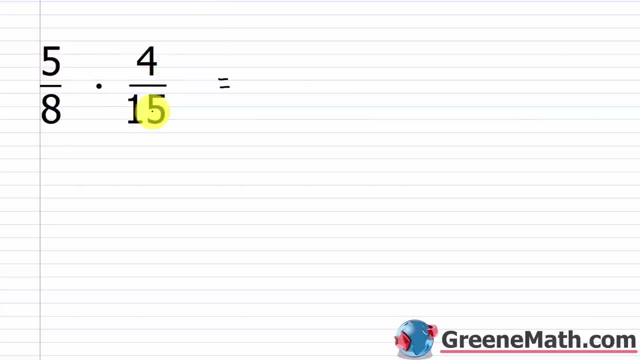 cancel, then I would look crossways. so I would look between 5 and 15. there's a common factor of 5, so 5 divided by 5 is 1, 15 divided by 5 is 3. and I look crossways again- between 8 and 4 there's a 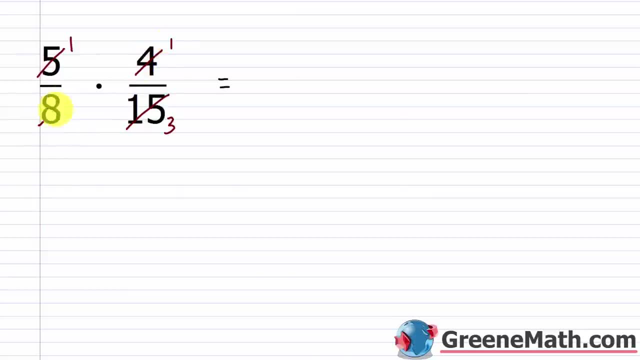 common factor of 4. so divide this by 4, I get 1, divide this by 4, I get 2.. so now, if I multiply 1 times 1, is 1, over 2 times 3, that's 6, so I get 1. 6th as the simplified form, or again reduced to its: 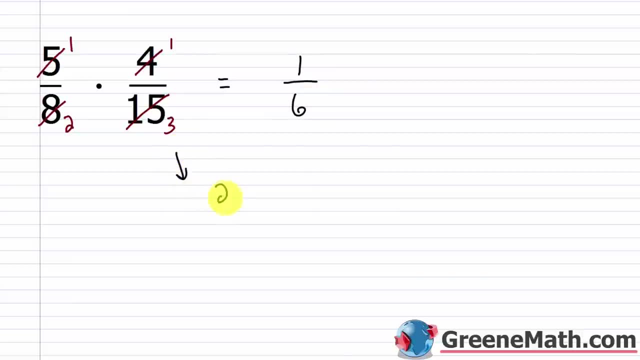 lowest terms. all right, so what about division? so recall that to divide one fraction by another, you take the first fraction. again, this division. now I've got to divide 1 by 6 and 4 into two. so find out the value of 8. here I can, AMT 10, put the whole denominator as the next argument to give me. 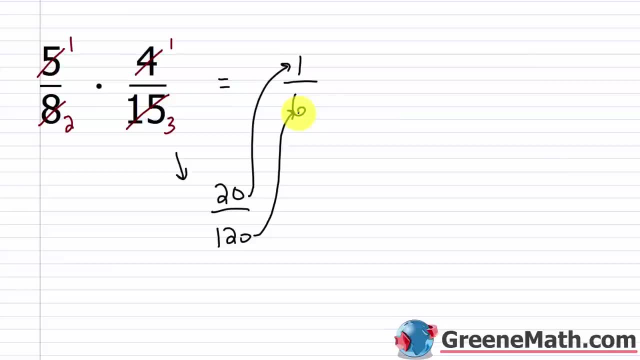 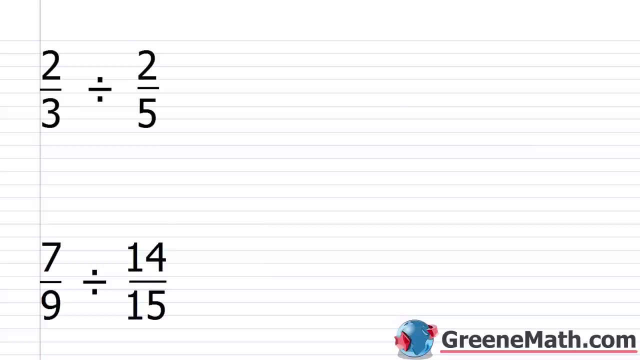 5 times 4, just like twice 10 minus 5 times 2, plus 10 times 8, plus 6 minus 8 minus 8. we're about half a point down into the denominator, so there's no significant difference. all right, so how do we divide all of these? so weчill get 10 divided by 5 and we'll see a little bit of that. unions with the equation. so the other way around we could do, and then you'll get a bit of this value. that's very much different because let's just so get to the exactly same error, so that the small normal distanceเศ training class where the drawn is 15 within the area of supercell is 20 times. 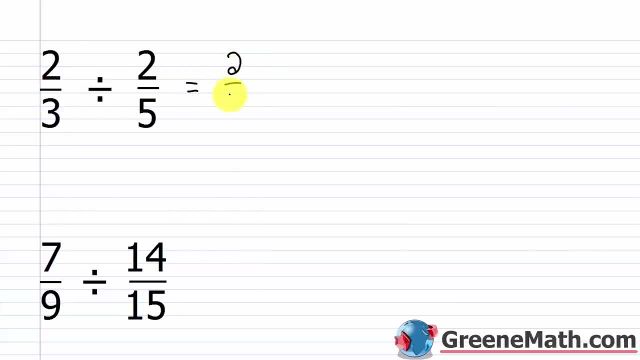 with a fraction all the way on the left and you leave that guy unchanged. then you change your division to multiplication and you're multiplying by the reciprocal of the second fraction. so if I take the reciprocal of two-fifths- remember I take the denominator and I bring it and put it into the numerator. 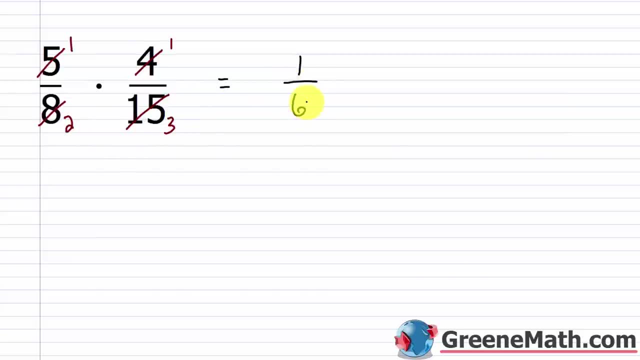 So I get 1 sixth as the simplified form, or again, reduced to its lowest terms. And again, if you wanted to do 5 times 4 and get... You know, 20 over 8 times 15, which is 120. So it's the same value, it just looks different. This is just unsimplified. 20 divided by 20 would give me 1, 120 divided by 20 would give me 6. So at the end of the day, you get 1 sixth, again, as the simplified form, or as they say, reduced to its lowest terms. 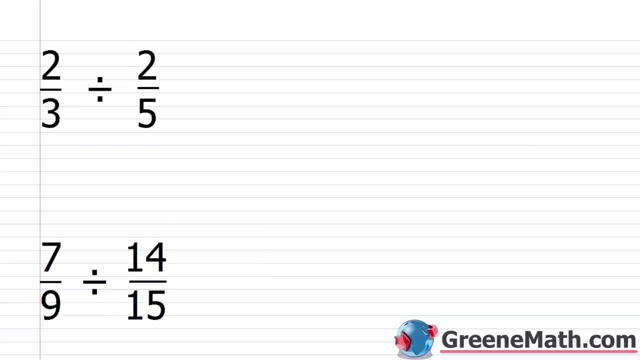 All right, so what about division? So recall that to divide one fraction by another, you take the first fraction, or the fraction all the way on the left. 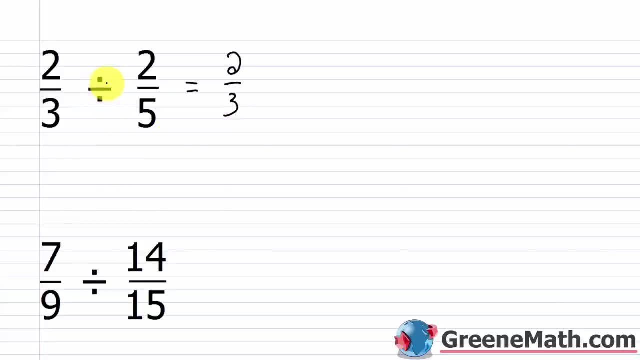 And you leave that guy unchanged. Then you change your division to multiplication. And you're multiplying by the reciprocal of the second fraction. 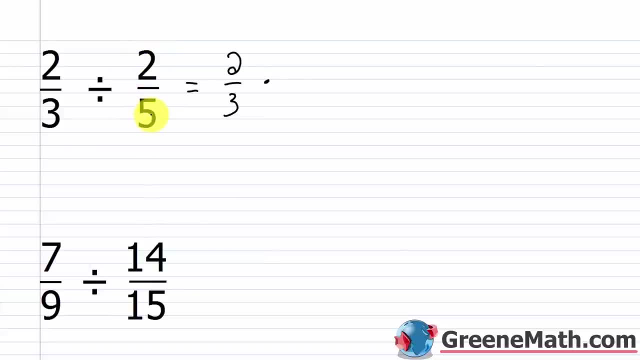 So if I take the reciprocal of 2 fifths, remember, I take the denominator, and I bring it and put it into the numerator, and I take the numerator, and I put it down into the denominator. So I just interchange or flip the positions. 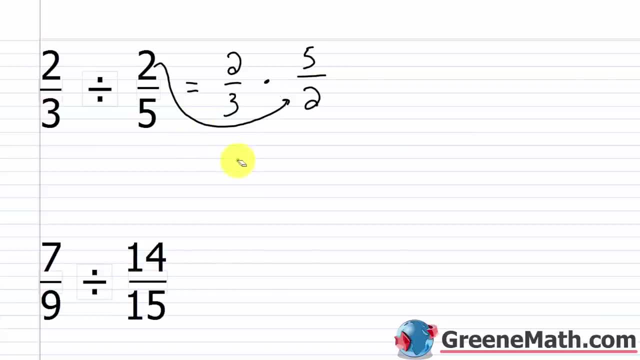 Denominator becomes numerator, numerator becomes denominator. So that's how you take the reciprocal. Now once I've done that, all I do is I just multiply. So I can see that I can cancel a common factor of 2 between here and here. So I'll put this as a 1 and this as a 1. And now I just multiply 1 times 5, that's 5, over 3 times 1, that's 3. So this is going to be 5 thirds. 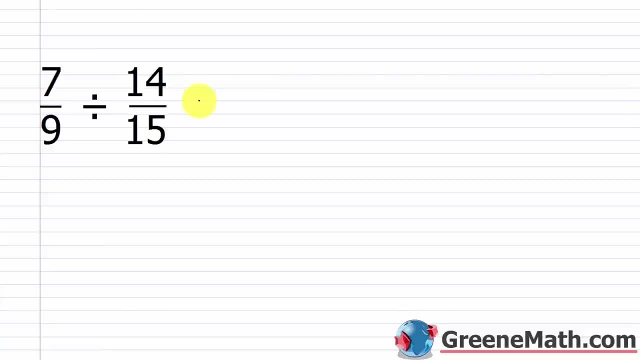 All right, so what about 7 ninths divided by 14 fifteenths? So I take 7 ninths, that's my fraction all the way to the left, I leave that unchanged. 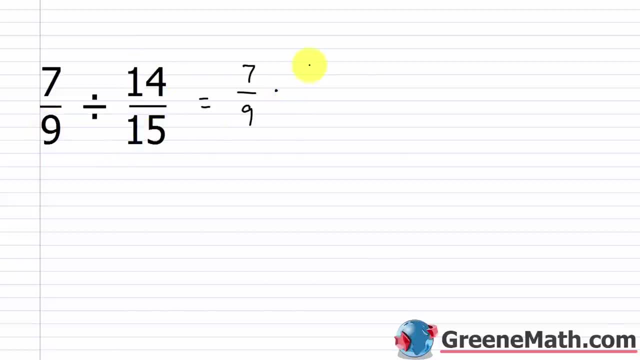 And I multiply this guy by the reciprocal of this. 15 goes into the numerator. 14 comes down into the denominator. So that's how you take the reciprocal. Again, this goes up here, this goes down there. You interchange. So now what can I cancel? Between 7 and 14, I have a common factor of 7. So this will be 2, and this will be 1. 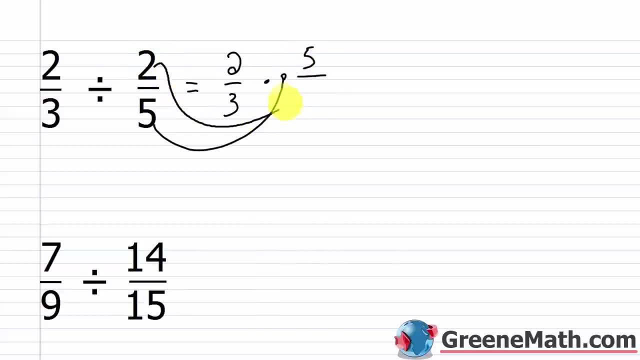 and I take the numerator and I put it down into the denominator, so I just interchange or flip the positions: denominator becomes numerator, numerator becomes denominator. so that's how you take the reciprocal. now, once I've done that, all I do is I just multiply so I can see that I can cancel a common. 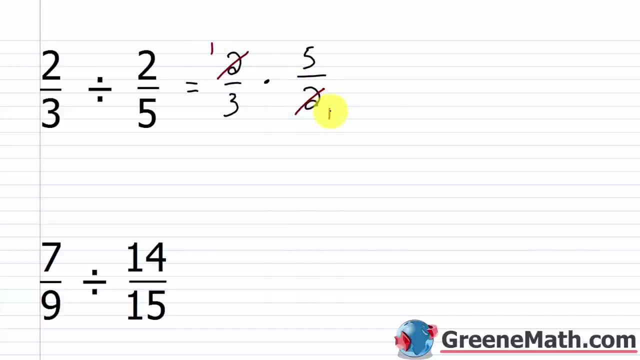 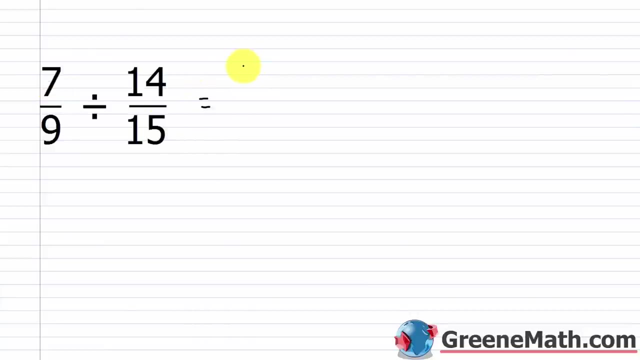 factor of two between here and here. so I'll put this as a 1 and this is a 1, and now I just multiply 1 times 5, that's 5. over 3 times 1, that's 3. so this is going to be 5 thirds. alright, so what about 7 9ths divided by 14 15ths? so I take 7. 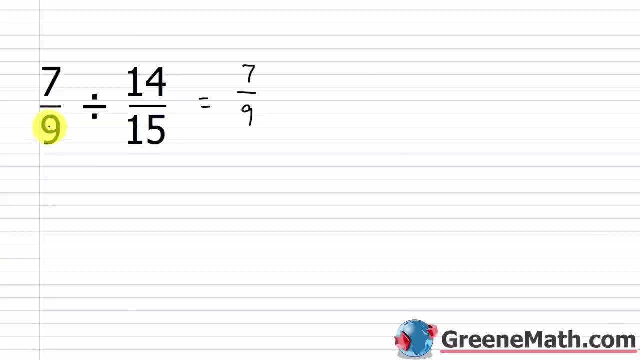 9ths. that's my fraction all the way to the left. I leave that unchanged and I multiply this guy by the reciprocal of the denominator and I multiply that by the reciprocal of this: 15 goes into the numerator, 14 comes down into the denominator. so that's how you take the reciprocal. again. this goes up here, this: 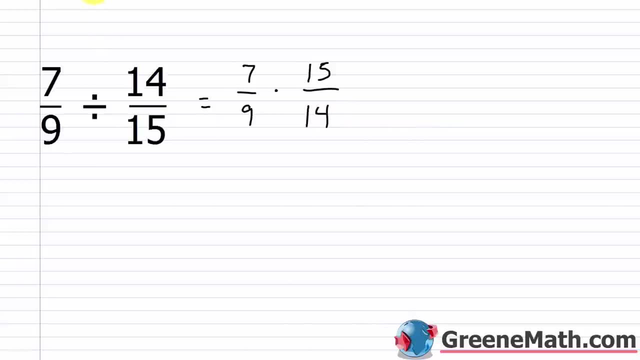 goes down. there you interchange. so now, what can I cancel? between 7 and 14, I have a common factor of 7, so this will be 2 and this will be 1. between 9 and 15: I have a common factor of 3, so this would be 3 and this would be 5. so now if 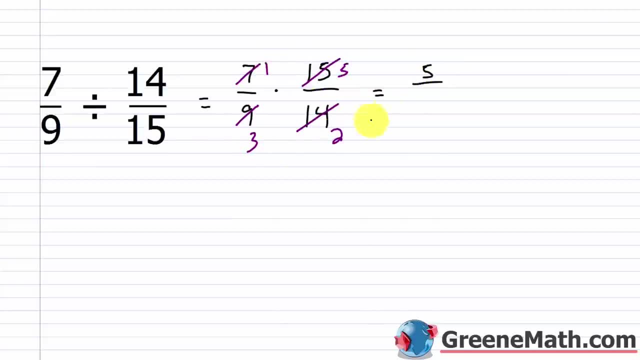 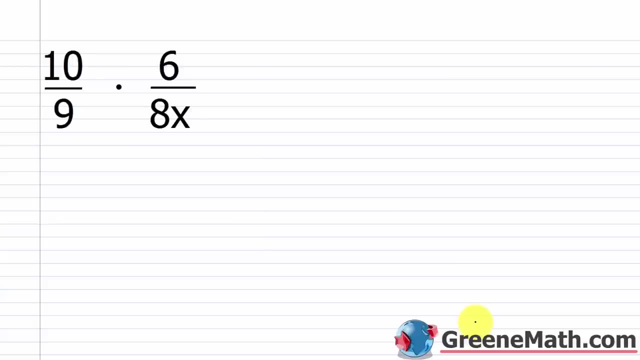 I multiply here: 1 times 5 is 5 over 3 times 2, that's 6. so we get 5, 6 as my answer. alright, so hopefully you're familiar with multiplying and dividing fractions. if you're not, at this point you might want to go back into a. 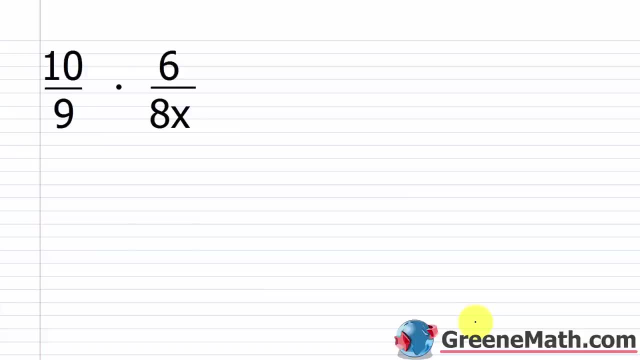 pre-algebra lesson on multiplying and dividing fractions. get up to speed on that and then come back to this point in the video. so now let's start looking at some rational expressions. if I had something like 10, 9 times 6 over 8 X, so 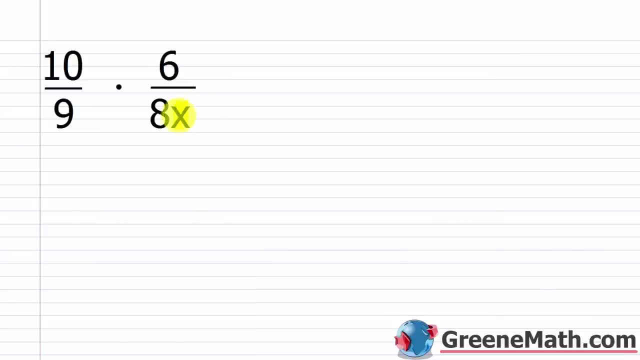 the only difference here is I have that one variable, which is X. nothing else is really going to change here. as far as the process, I'm still going to look to cross cancel before I start my multiplication. so what are the common factors between 10 and 9? you can't really cancel anything there. 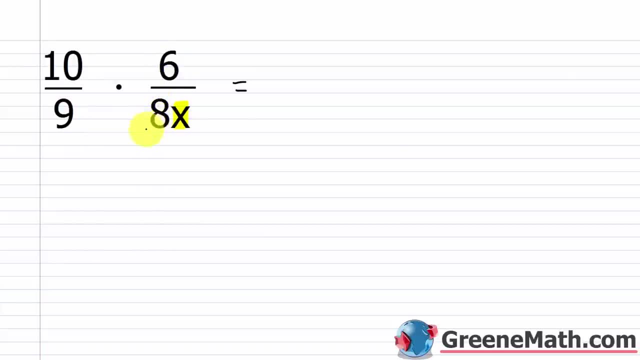 between 6 and 8, I can cancel a common factor of two, so I can make this a 4X and I can make this a 3. now I can do more canceling because I can cross cancel between this 9 and this 3. so if I divide this by 3, I get 3. if I divide 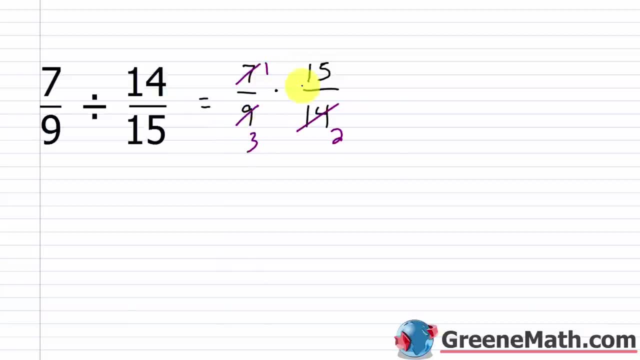 Between 9 and 15, I have a common factor of 3. So this would be 3, and this would be 5. So now if I multiply here, 1 times 5 is 5, over 3 times 2, that's 6. So I get 5 sixths as my answer. 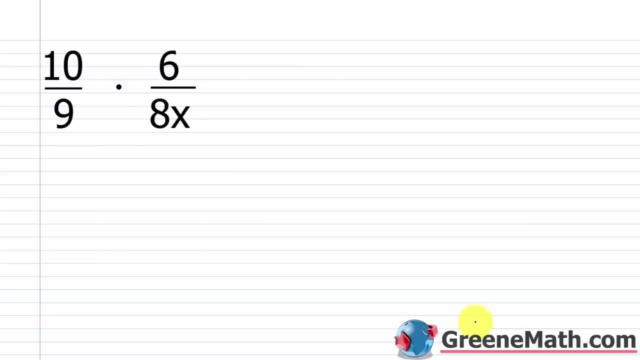 Hopefully you're familiar with multiplying and dividing fractions. If you're not at this point, you might want to go back into a pre-algebra lesson on multiplying and dividing fractions. Get up to speed on that, and then come back to this point in the video. 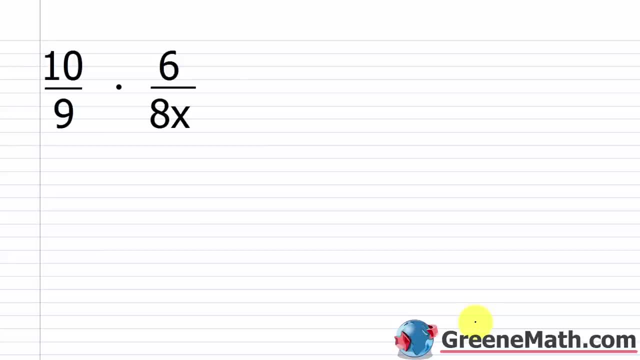 So now let's start looking at some rational expressions. If I had something like 10 ninths times 6 over 8x. 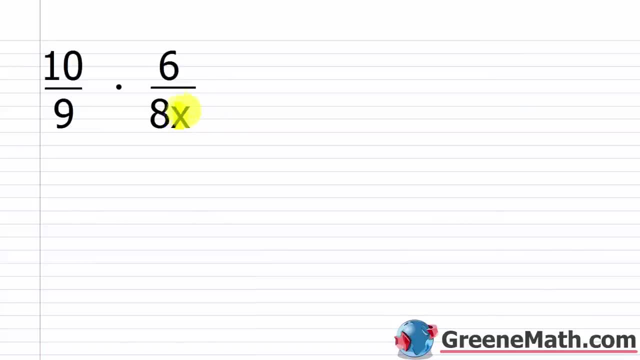 So the only difference here is I have that one variable, which is x. Nothing else is really going to change here. As far as the process. 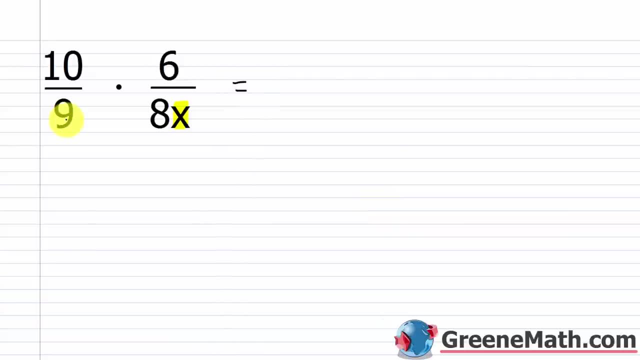 I'm still going to look to cross cancel before I start my multiplication. So what are the common factors between 10 and 9? Can't really cancel anything there. Between 6 and 8, I can cancel a common factor of 2. 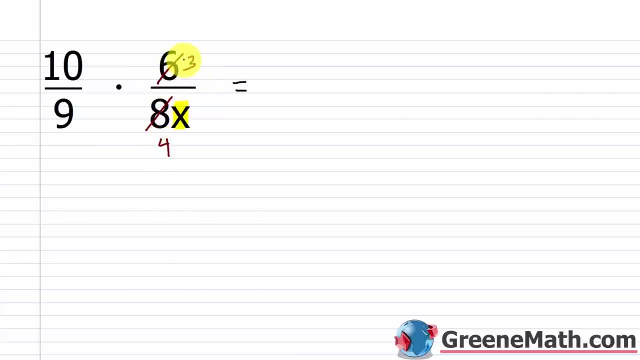 So I can make this a 4x, and I can make this a 3. Now I can do more canceling, because I can cross cancel between this 9 and this 3. So if I divide this by 3, I get 3. If I divide this by 3, I get 1. Then I can do some more cross canceling. Because 10 is divisible by 2, and so is 4. 10 divided by 2 is 5. 4 divided by 2 is 2. So now we just multiply. 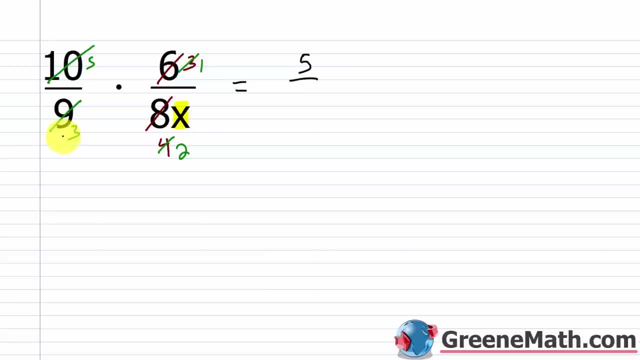 5 times 1 is 5. Over 3 times 2x. 3 times 2 is 6. And then x comes along for the ride. So we get 5 over 6x. 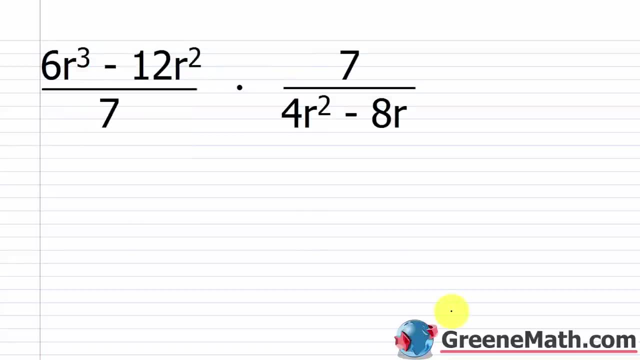 Alright, so that was pretty easy. Let's look at one that's a little bit more complicated. 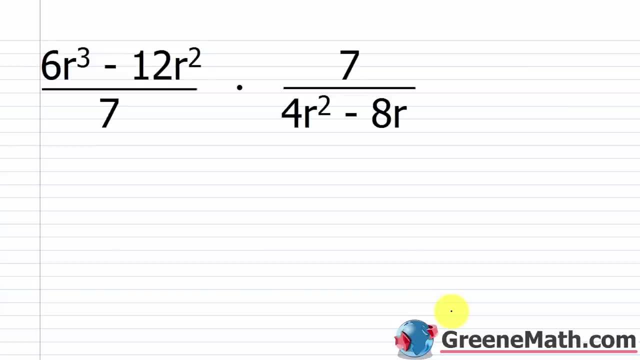 So we have 6r cubed minus 12r squared. This is over 7. 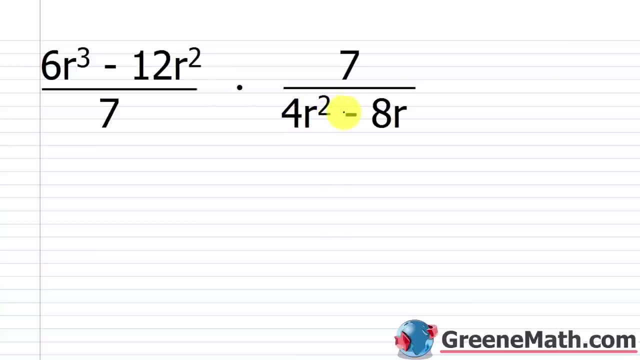 And then we're multiplying by 7 over 4r squared minus 8r. 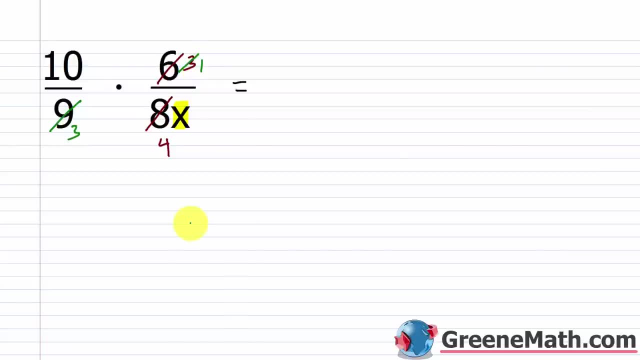 this by 3, I get 1. do some more cross canceling, because 10 is divisible by 2 and so is 4.. 10 divided by 2 is 5.. 4 divided by 2 is 2.. So now we just multiply: 5 times 1 is 5 over 3 times 2x. 3 times 2 is 6. 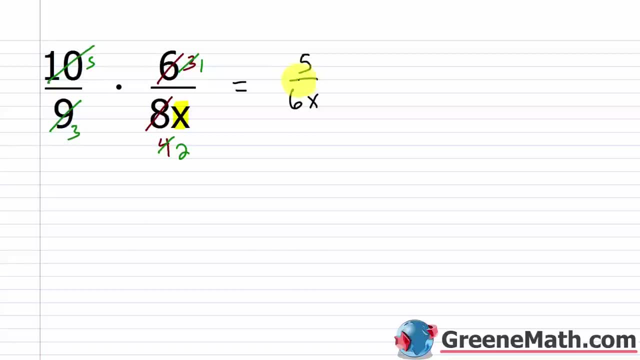 and then x comes along for the ride. So we get 5 over 6x. All right, so that was pretty easy. Let's look at one that's a little bit more complicated. So we have 6r cubed minus 12r squared. This is: 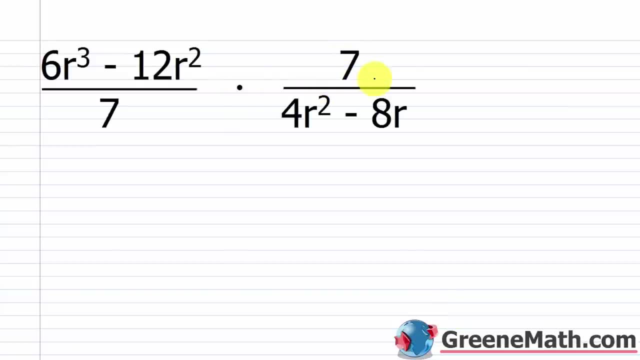 over 7, and then we're multiplying by 7 over 4r, squared minus 8r. So the trick to this is the first thing you want to do is you want to factor out the greatest common factor from every numerator and every denominator. Now, before I even do that, I notice that I can cancel this 7 with. 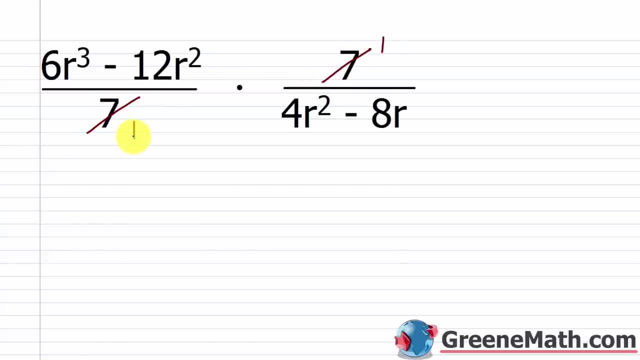 this 7.. I can cross cancel. so this is a 1 and this is a 1.. Now if I kind of factor out the GCF here in the numerator over here, it would be a 6r squared. So I can write 6r squared times the quantity. I would just have an r minus a 2.. 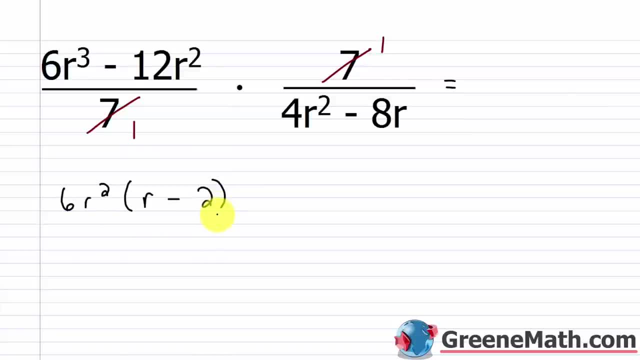 Now this is over 1, so I can write it over 1 or I can leave it as it is. It doesn't really matter, because I have a numerator and denominator here. Let me just write it over 1, kind of to make things consistent. So times: here I have a 1 over The GCF, here is 4r, so I'm going to write this as: 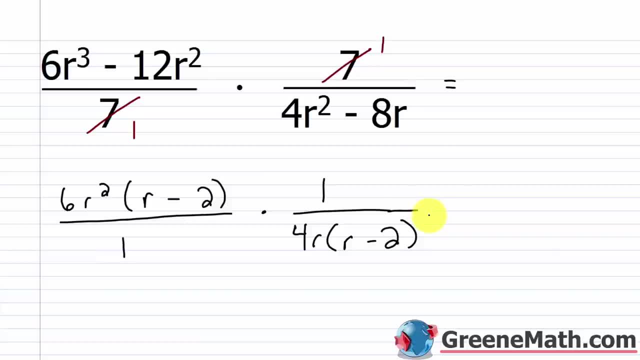 the denominator over here is this: OK, I want to say this is a 5 over 6 and this is a 1 over 2.. But remember what else I can cancel. What else can I cancel? and there's two things I can cancel. 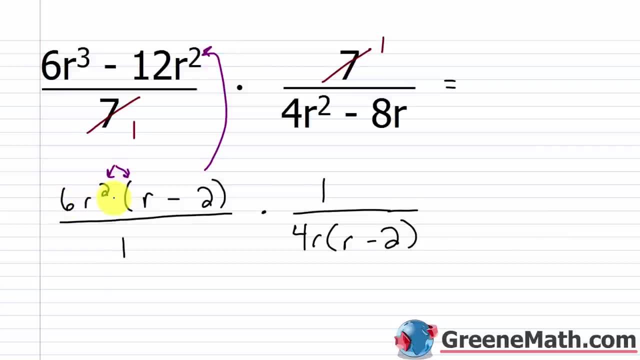 The first thing is that I have a common factor: of r minus 2.. Remember these two here are factors. They are being multiplied together to give me this 6r squared times the quantity r minus 2.. So they are factors, Ok. 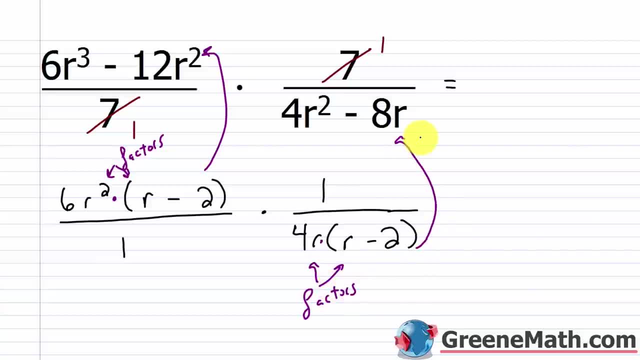 Remember that would combine to give me four R squared minus eight R. So I can cancel common factors, So I can cancel this with this and that would give me a one and a one. Now, in addition to that, I can do some more canceling What I can do: six and four each divisible by two If I divide this. 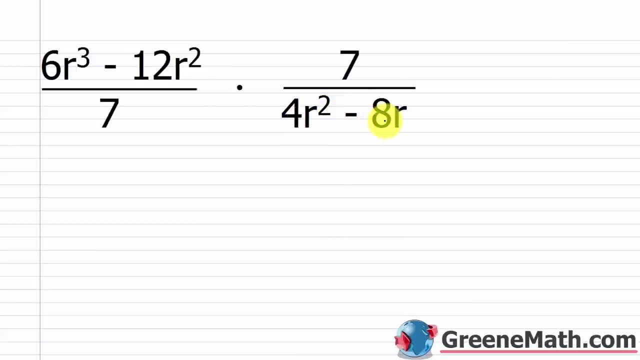 So the trick to this is, the first thing you want to do is you want to factor out the greatest common factor from every numerator and every denominator. Now, before I even do that, I notice that I can cancel this 7 with this 7. I can cross cancel. So this is a 1, and this is a 1. Now, if I kind of factor out the GCF here, in the numerator over here, it would be a 6r squared. So I can write 6r squared times the quantity. I would just have an r minus a 2. Now, this is over 1, so I can write it over 1, or I can leave it as it is. It doesn't really matter. 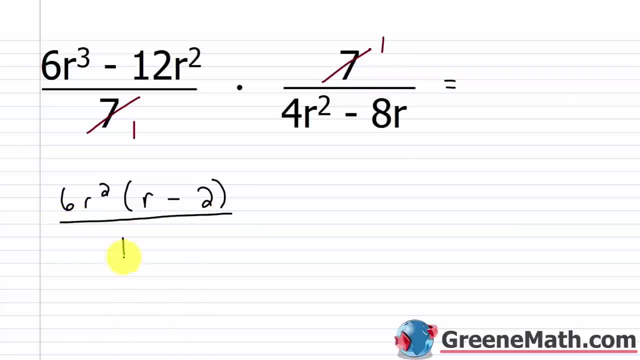 Because I have a numerator and a denominator here, let me just write it over 1. Kind of to make things consistent. So times, here I have a 1 over. The GCF here is 4r. So I'm going to write this as r minus 2 as well. Now. 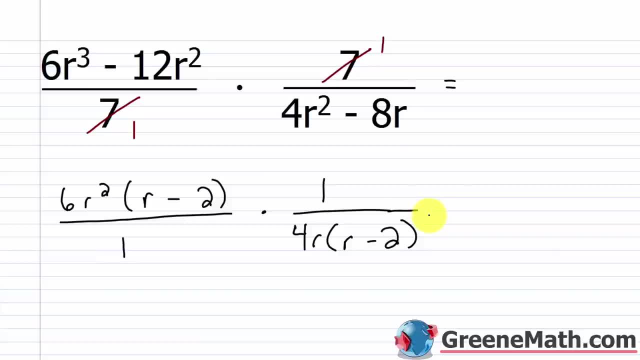 What else can I cancel? And there's two things I can cancel. 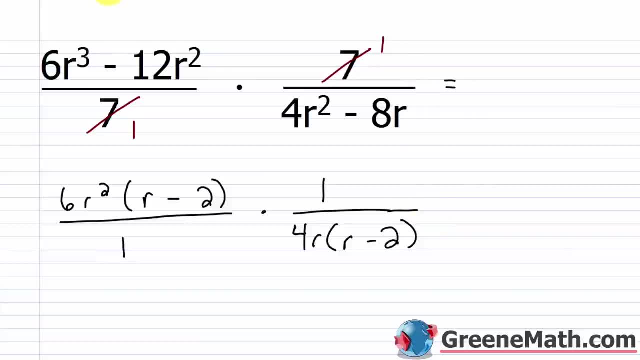 The first thing is that I have a common factor of r minus 2. Remember, these two here are factors. 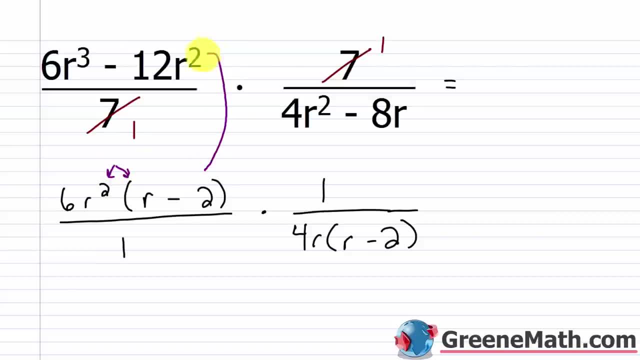 They are being multiplied together to give me this. 6r squared times the quantity r minus 2. So they are factors. 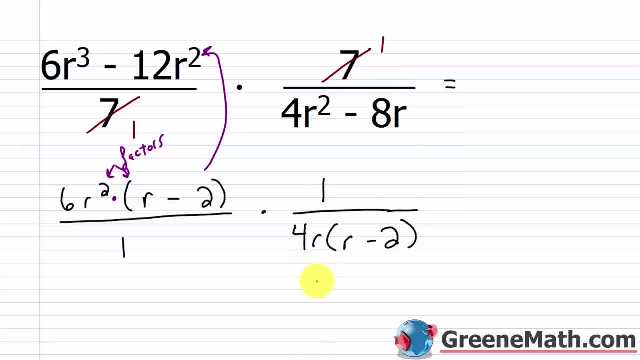 Okay, remember that. Over here I have factors. 4r is being multiplied by r minus 2. These are factors. 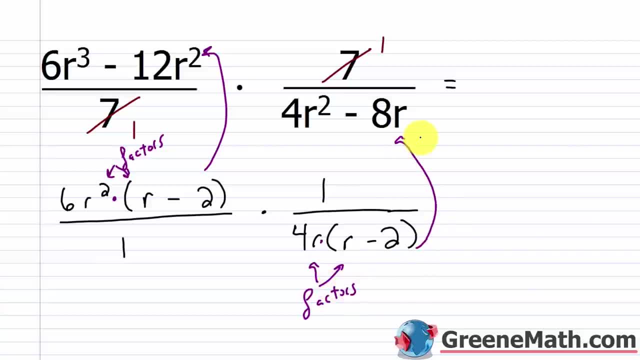 And that would combine to give me 4r squared minus 8r. So I can cancel common factors. So I can cancel this with this. And that would give me a 1 and a 1. Now, in addition to that, I can do some more cancelling. What I can do, 6 and 4 each divisible by 2. If I divide this by 2, I get a 3. If I divide this by 2, I get a 2. Then I can also cancel one common factor of r. 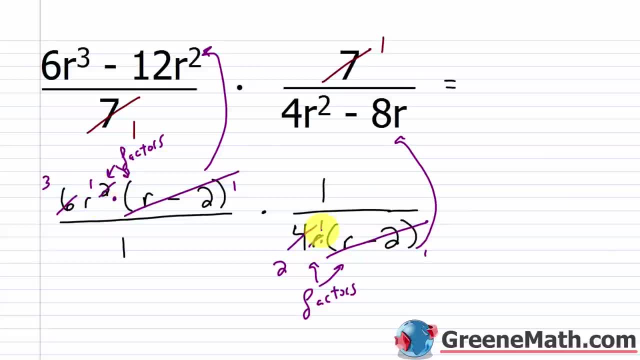 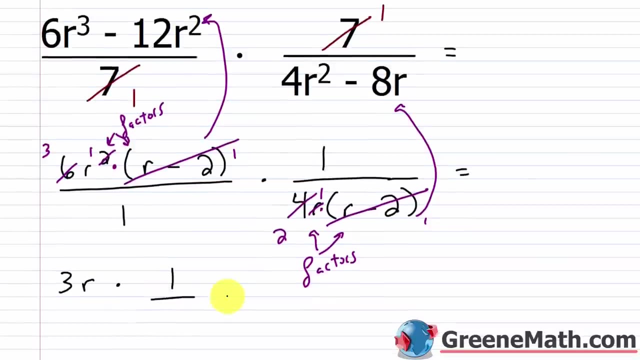 So this would be r to the first power. And this would just be a 1. So what I'd end up with, let me put equals here. I would have 3r. Everything else is a 1. It's times 1 and it's over 1. So then times, over here I'd have 1 over. I'd have 2. 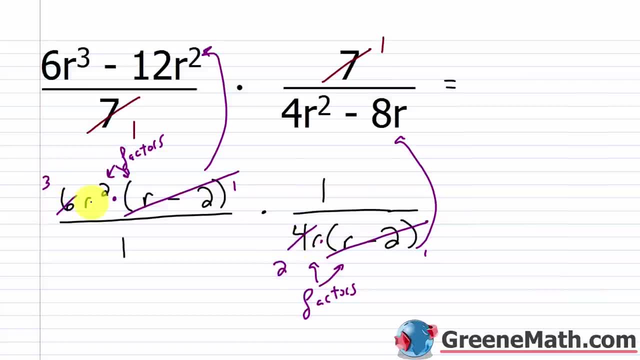 by two, I get a three. If I divide this by two, I get a two. Then I can also cancel one common factor of R. So this would be R to the first power and this would just be a one. So what I'd? 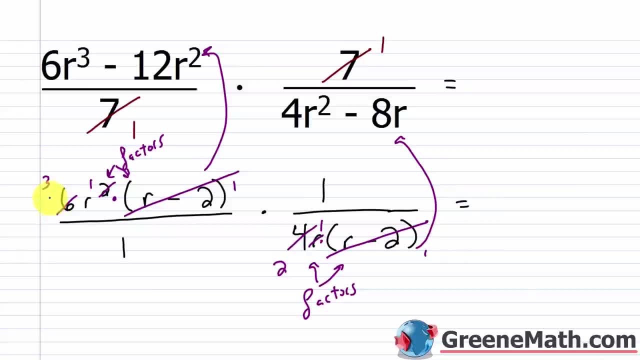 end up with- let me put equals here. I would have three R. Everything else is a one, It's times one and it's over one. So then, times over here. I'd have one, over I'd have two. Everything else is. 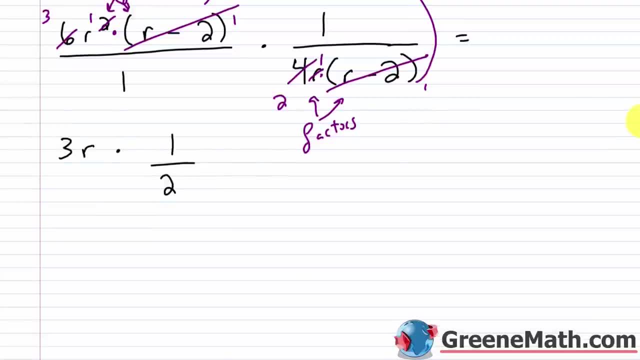 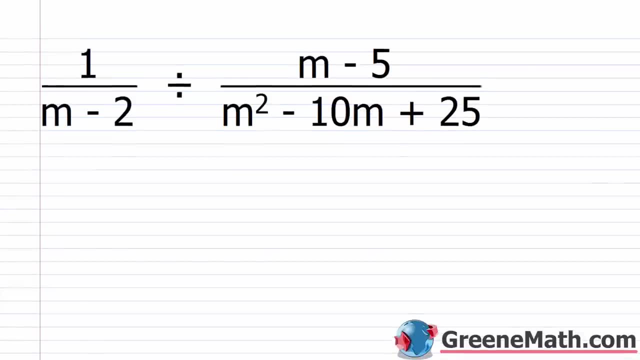 a one. So essentially, when I write my answer here, this is going to be equal to three R over two. So just three R over All. right, let's take a look at another one. So we have one over M minus two, and this is divided. 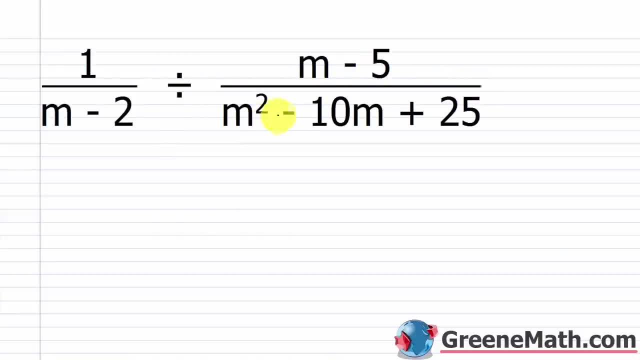 by M minus five over M squared minus 10M plus 25.. Okay, So the first thing I want to do is set this up. Remember, if I'm dividing, just like if I'm dividing with fractions, the first guy over here. 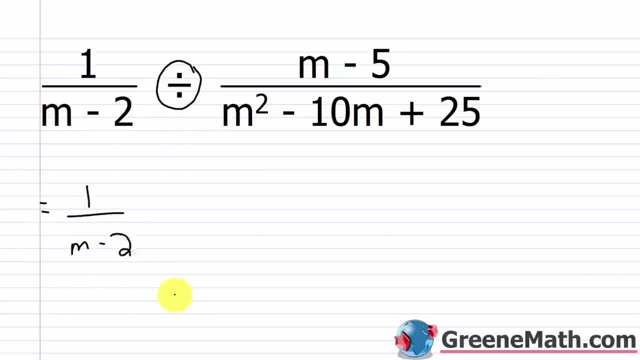 is going to stay the same. So one over M minus two. Then I'm going to multiply by the reciprocal of this. So this is going to go on: the numerator M squared minus 10M plus 25.. And then this is going to go on. 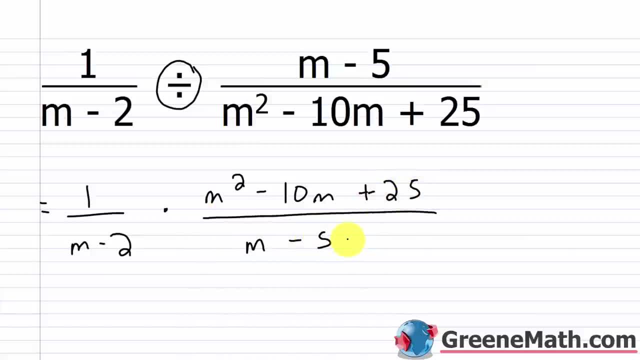 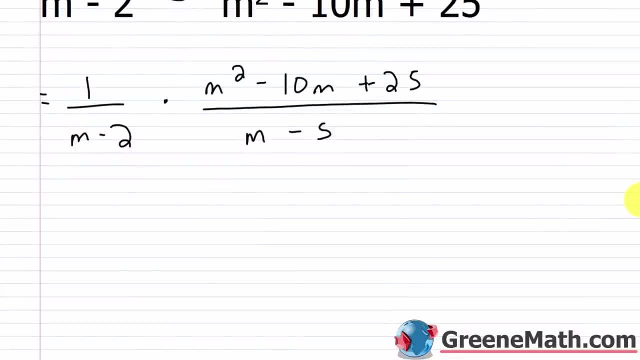 the denominator M minus five. Now let's take a look at factoring the top. So we need two integers whose sum is negative 10 and whose product is 25.. Well, negative five and negative five would be those two integers. So let's write: equals one over M minus two. 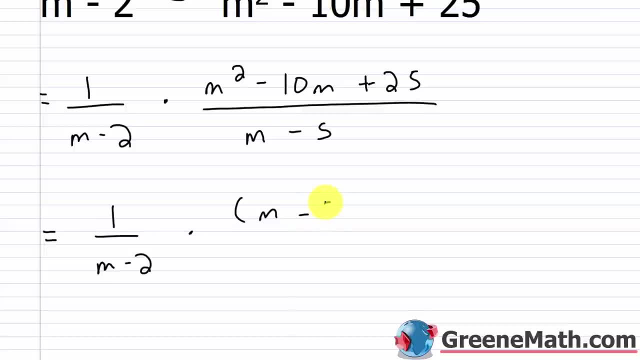 I'm going to factor this into M minus five times M minus five, And obviously I can cancel that with M minus five down here. And to make this obvious when you first start doing it, you can just write this as times one, right, Anything times one. So you can say: this is a. 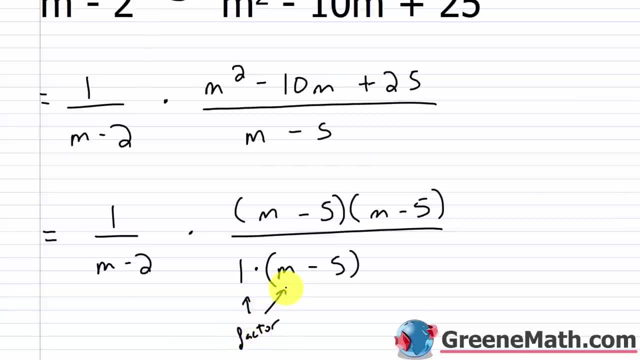 factor, And so is this. So it's one times that, All right. So we cancel common factors, cancel this with this, And what I'm left with is: what do I get? I get this, I get this, I get this, I get. Everything else is a 1. 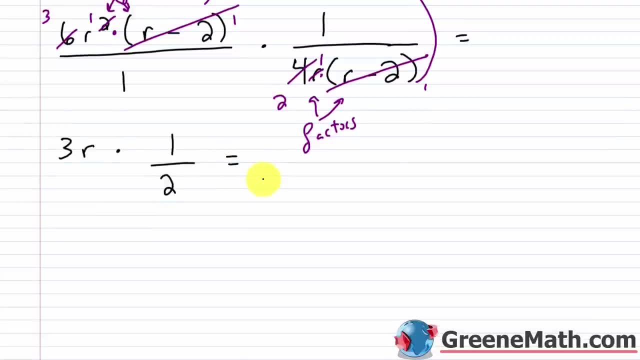 So essentially, when I write my answer here, this is going to be equal to 3r over 2. So just 3r over 2. Alright, let's take a look at another one. 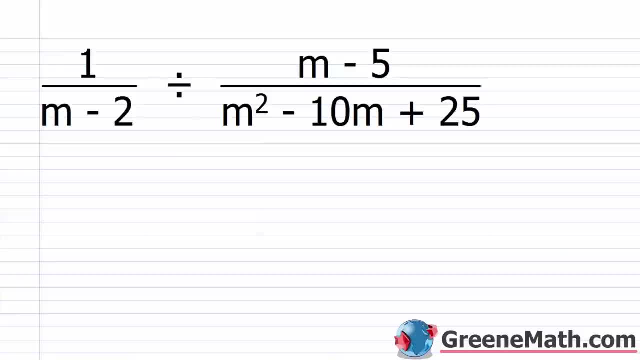 So we have 1 over m minus 2. And this is divided by m minus 5 over m squared minus 10m plus 25. 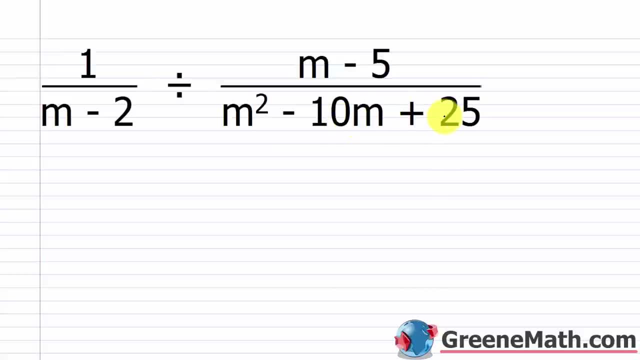 So the first thing I want to do is set this up. Remember, if I'm dividing, just like if I'm dividing with fractions, the first guy over here is going to stay the same. So 1 over m minus 2. 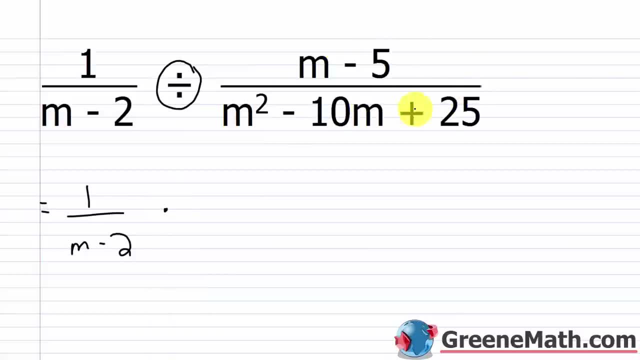 Then I'm going to multiply by the reciprocal of this. So this is going to go on the numerator. 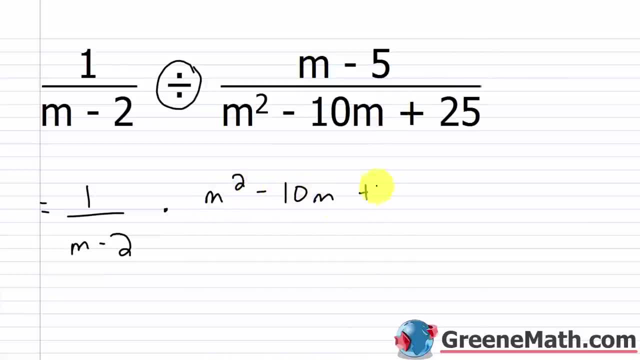 m squared minus 10m plus 25. And then this is going to go on the denominator. m minus 5. 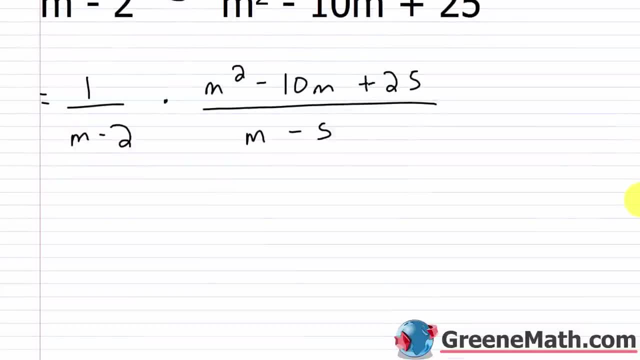 Now, let's take a look at factoring the top. So we need two integers whose sum is negative 10 and whose product is 25. Well, negative 5 and negative 5 would be those two integers. So let's write equals 1 over m minus 2. 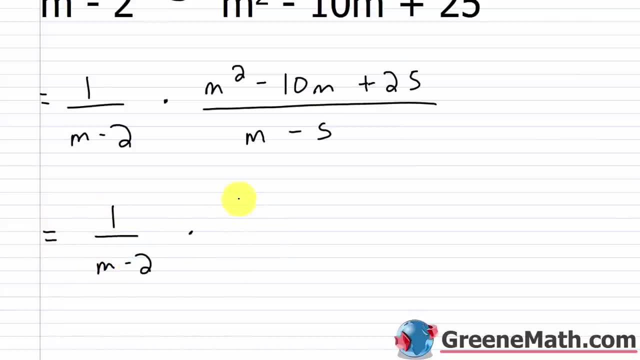 m minus 2 times, I'm going to factor this into m minus 5 times m minus 5. And obviously, I can cancel that with m minus 5 down here. And to make this obvious when you first start doing it, you can just write this as times 1. Anything times 1. So you can say this is a factor and so is this. So it's 1 times that. Alright, so we cancel common factors. Cancel this with this. 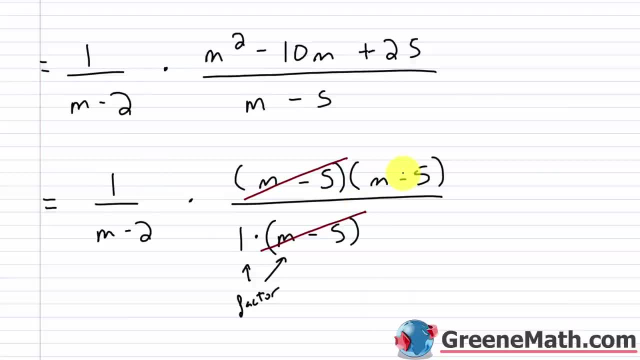 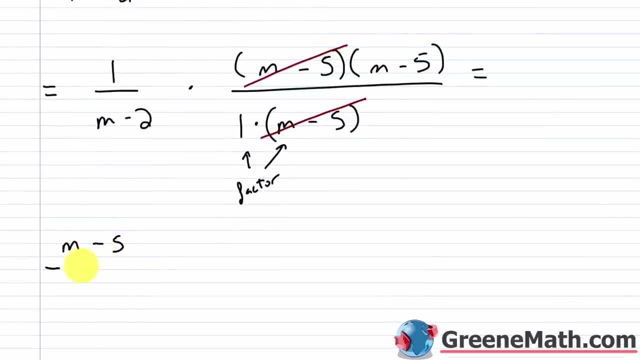 And what I'm left with is 1 times m minus 5 in the numerator. Let me scroll down here. That would be m minus 5. And this is over m minus 2 times 1, which is just m minus 2. 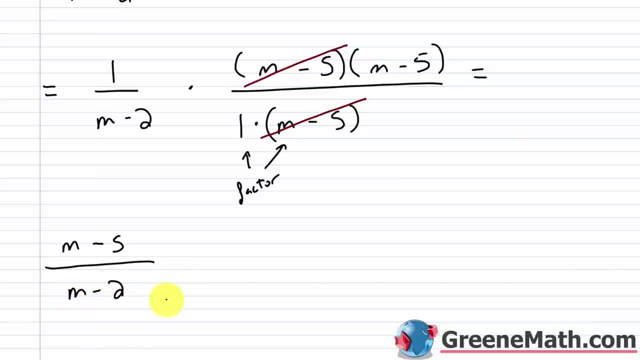 So my simplified answer here is m minus 5 over m minus 2. 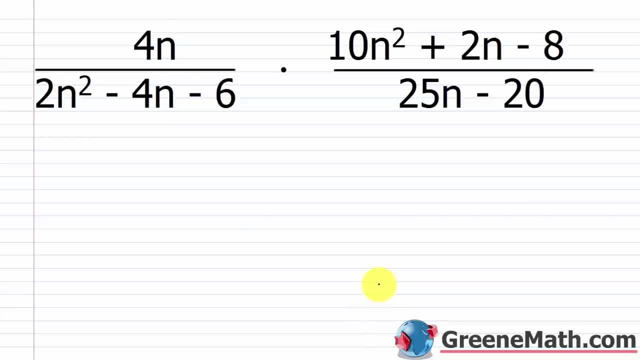 Okay, let's take a look at another one that's a little bit more tedious. 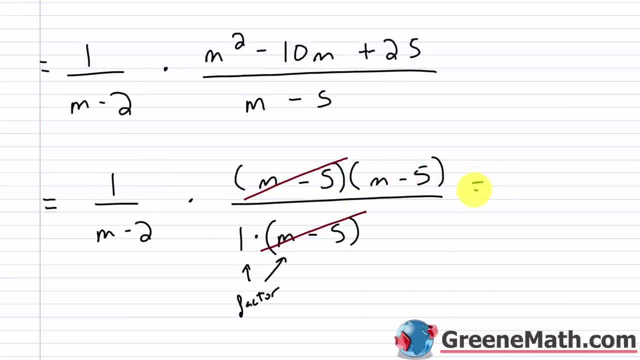 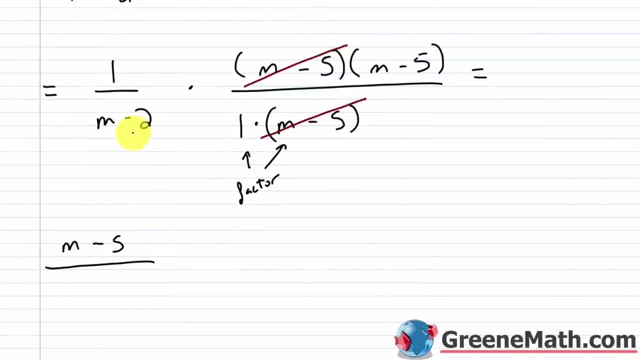 is 1 times m minus 5. in the numerator Let me scroll down here- That would be m minus 5 and this is over m minus 2 times 1, which is just m minus 2.. So my simplified answer here is m minus. 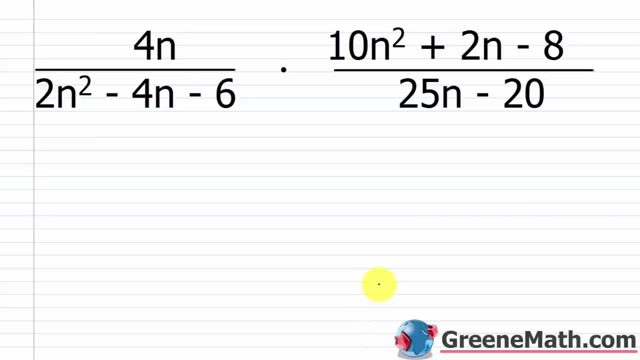 5 over m minus 2.. Okay, let's take a look at another one that's a little bit more tedious. So we have 4n over 2n squared minus 4n minus 6 times 10n squared plus 2n minus 8, and this is: 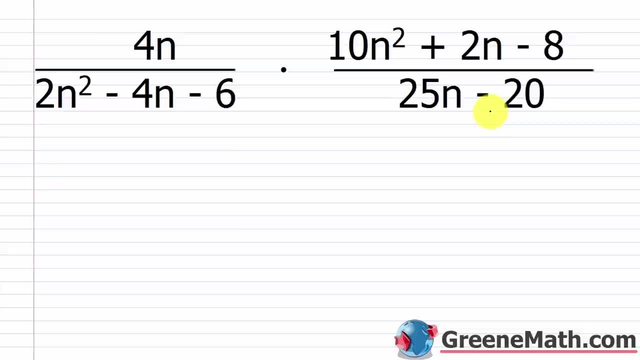 over 25n minus 20.. So all I'm going to do is just factor everything completely or as much as I need to, to figure out what's going to cancel. So, for example, in this numerator here, 4n, I'm not going to write 2 times, 2 times n, I'm just going to write 4n. You can do that if you want, but I think 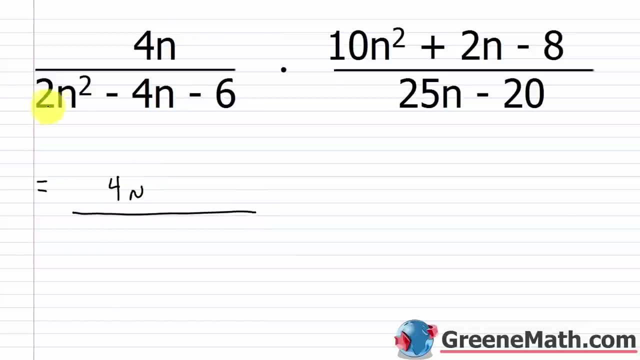 it's a bit unnecessary. So then over here you have 2n squared minus 4n minus 6.. So I'm going to start by just pulling a 2 out of there, and that would give me n squared minus 2n minus 6.. So I'm going to start by just pulling a 2 out of there, and that would give me n squared minus 2n. 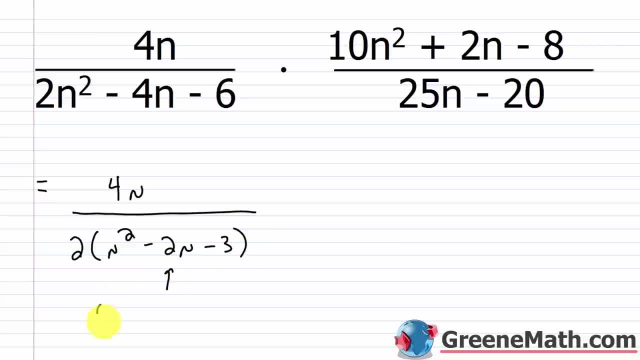 minus 6.. So I'm going to start by just pulling a 2 out of there, and that would give me n squared minus 2n minus 3.. Now I can further factor this, So this would be n and then n, So give me two integers. 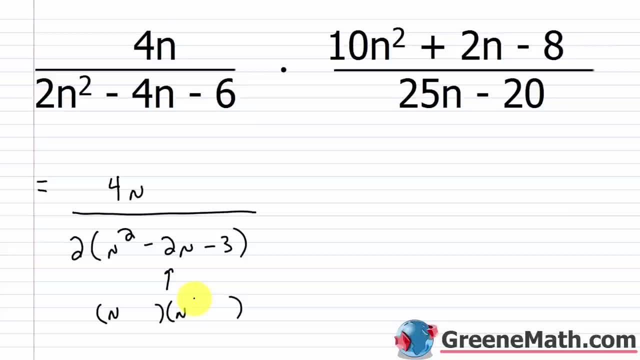 whose sum is negative 2 and whose product is negative 3. So that would be negative 3 and positive 1.. So let me erase this part and I'll drag this up here, Okay. So then this is times Up here I have 10n squared plus 2n minus 8. So let me factor that. 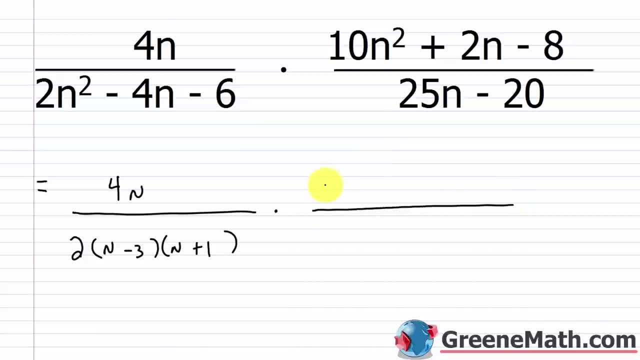 at the bottom because I need a little room for that. I'm just going to start by just putting okay two times If I pull a 2 out of there, because it's common to everything: 5n squared plus n minus 4.. Then over here, 25n minus 20.. I can pull a 5 out And that's going to be. 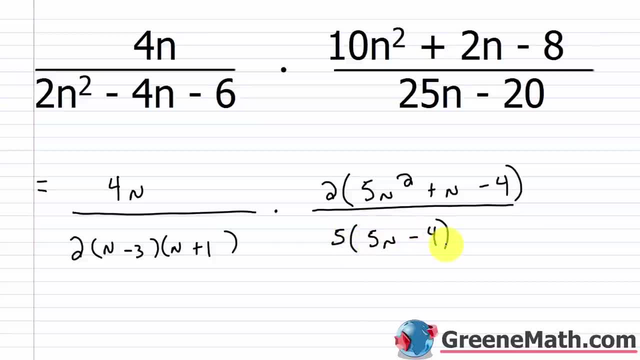 5n squared plus n minus 4.. So that's going to be 5n squared plus n minus 4.. And then over here 25n. that's going to give me 5n minus 4.. Now let me just factor this guy down here. so I have a little. 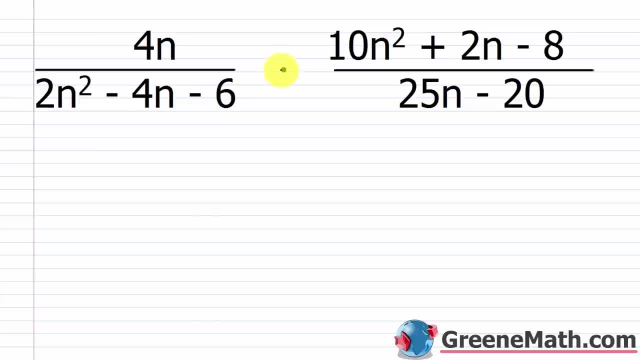 So we have 4n over 2n squared minus 4n minus 6 times 10n squared plus 25. This is 2n minus 8. 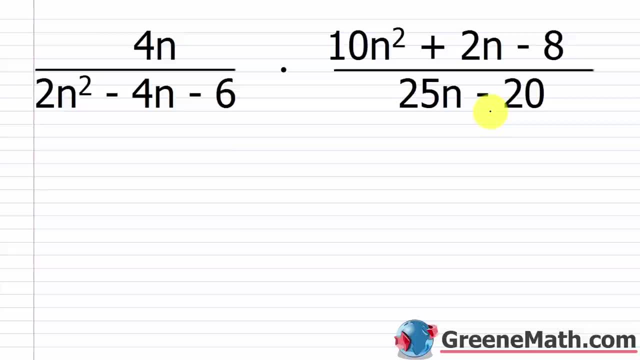 And this is over 25n minus 20. So all I'm going to do is just factor everything completely or as much as I need to to figure out what's going to cancel. 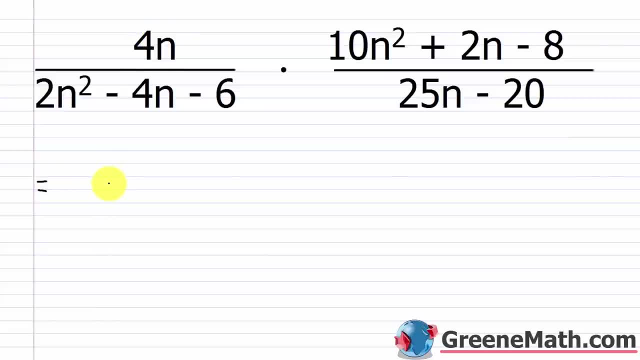 So, for example, in this numerator here, 4n, I'm not going to write 2 times 2 times n. I'm just going to write 4n. 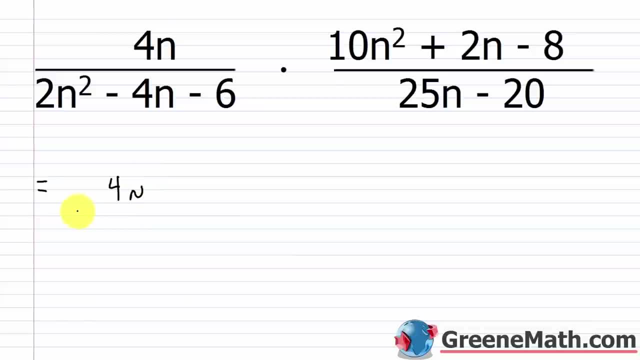 You can do that if you want, but I think it's a bit unnecessary. So then over, here you have 2n squared minus 4n minus 6. So I'm going to start by just pulling a 2 out of there. 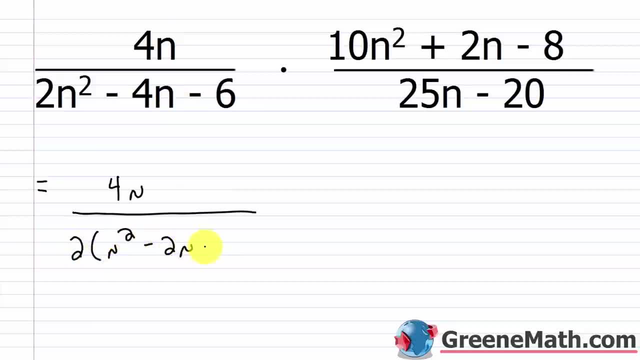 And that would give me n squared minus 2n minus 3. Now I can further factor this. So this would be n and then n. So give me two integers whose sum is negative 2 and whose product is negative 3. So that would be negative 3 and positive 1. 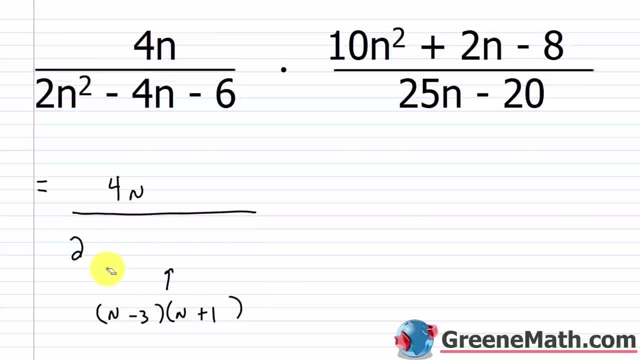 So let me erase this part and I'll drag this up here. 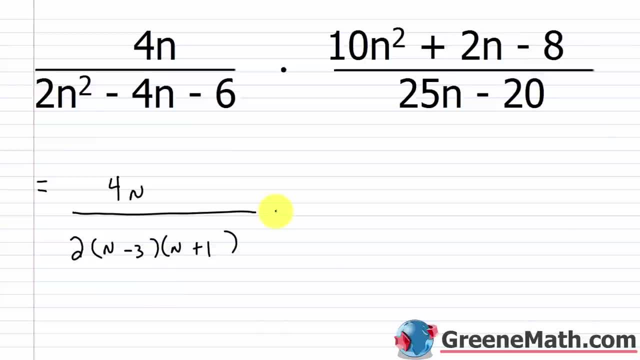 Okay, so then this is times. Up here I have 10n squared plus 2n minus 8. 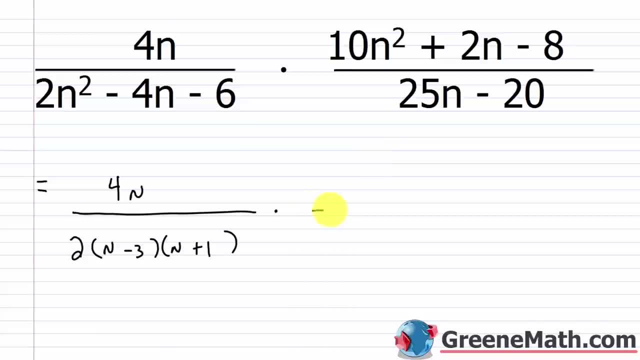 So let me factor that at the bottom because I need a little room for that. I'm just going to start by just putting, okay, 2 times, if I pull a 2 out of there because it's common to everything, 5n squared plus n minus 4. Then over here, 25n minus 20. I can pull a 5 out and that's going to give me 5n minus 4. Now let me just factor this guy down here so I have a little room. 5n squared plus n minus 4. 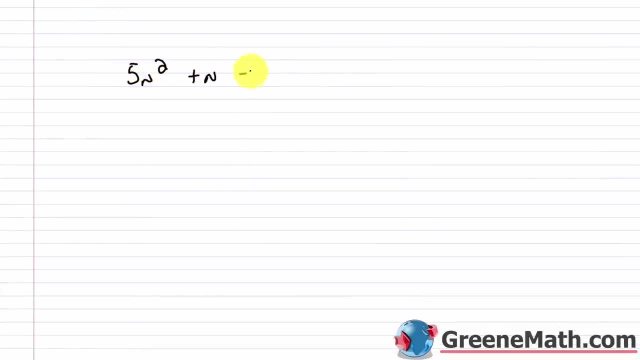 So 5n squared plus n minus 4. 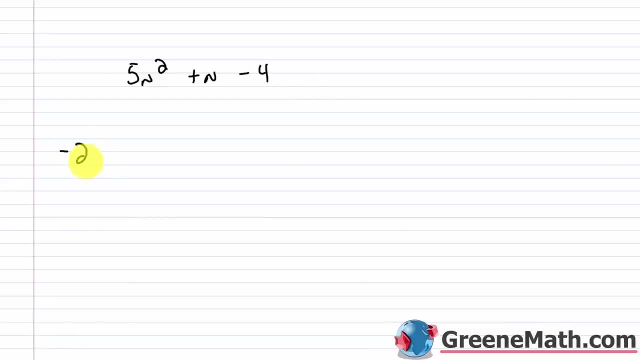 So I need two integers whose product is negative 20 for the product. 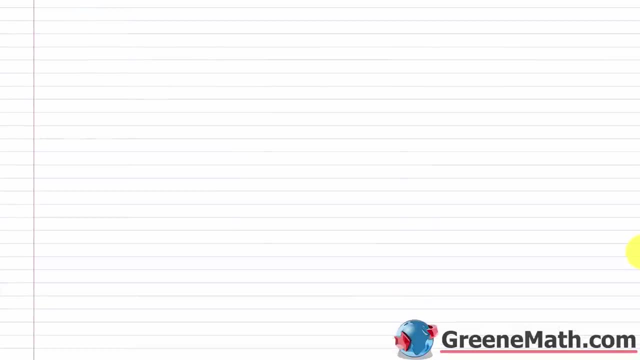 room: 5n squared plus n minus 4.. So 5n squared plus n minus 4.. So I need two integers whose product is negative, 20 for the product, and then I need a sum of 1.. So for 20, forget about the. 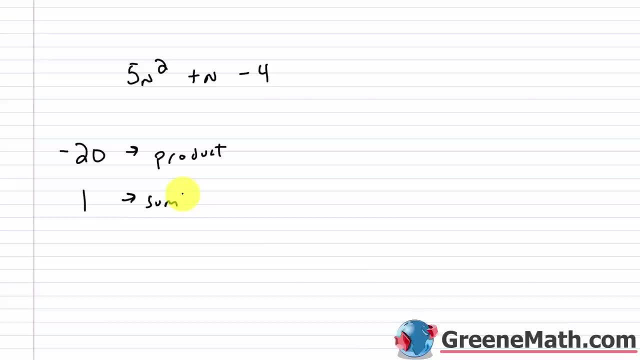 negative for a minute. I know 5 times 4, so I can play with that and get a sum of 1.. If I had positive 5 and negative 4, that would work out. So let's use those So we would have. this is equal to. 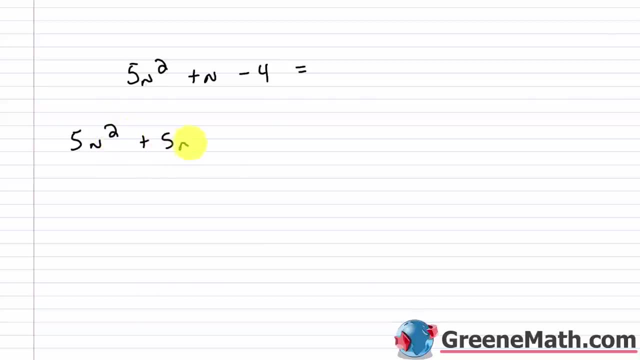 5n squared plus 5n minus 4n minus 4.. If we factor this by grouping, I could pull a 5n out of the first group. That would leave me with an n plus 1 here. Out of the second group I can pull out a negative 4. That would leave me with n plus 1 here. So the 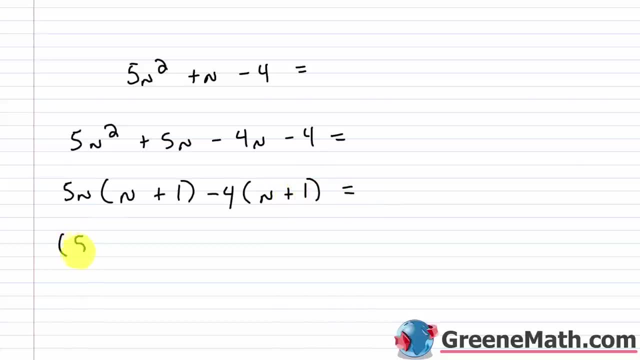 common binomial factor is n plus 1.. So I would have 5n minus 4, that quantity, times n plus 1, that quantity. So that's your factored form, All right, so let's erase this real quick. We'll put that. 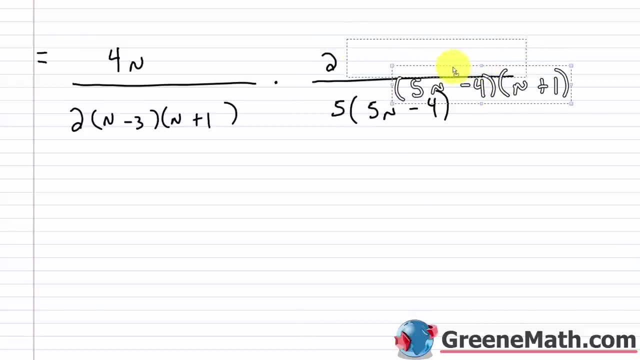 factored form in here. Nice and convenient, Okay. so now what we want to do is we want to look to see what we can cancel. We have everything that's factored, as much as we need to, And so I see that I have a common factor of 5n minus 4.. Again, this is multiplication here. 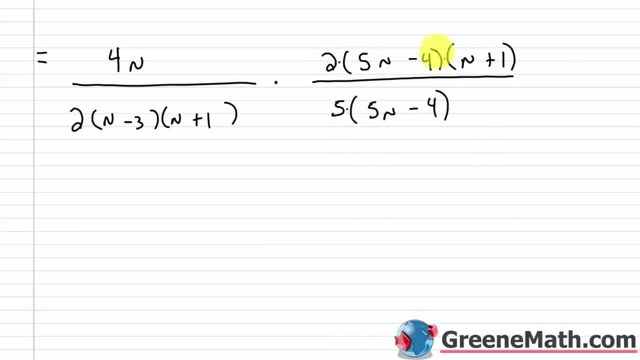 Everything is being multiplied. This is multiplication. So these are all factors. So this factor of 5n minus 4 will cancel with this factor of 5n minus 4.. This factor of n plus 1 will cancel with this factor of n plus 1.. We can cancel this 2 with. 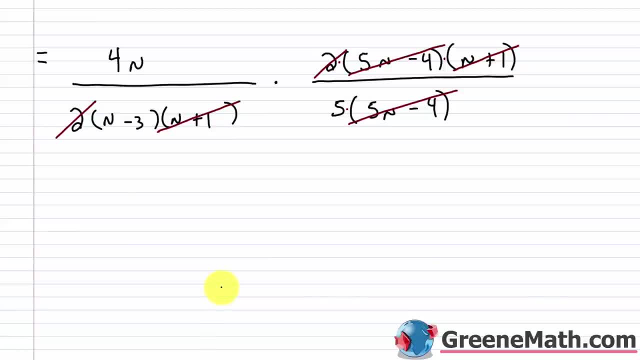 this 2.. And is there anything left that I can cancel? There's nothing up here other than a 1.. Remember: when your numerator or your denominator cancels completely, you write a 1.. Down here I just have a 5.. So I need to be able to cancel a 5 with something over here I can't. So that's simplified. 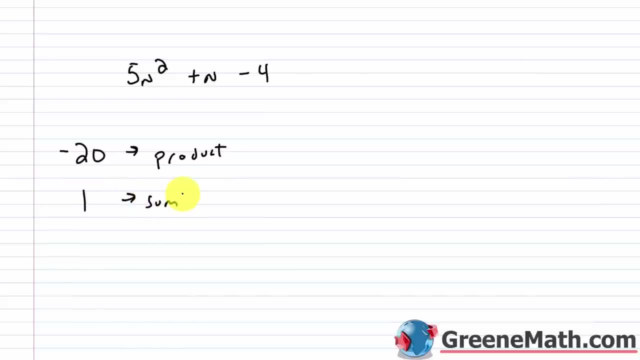 And then I need a sum of 1. So for 20, forget about the negative for a minute, I know 5 times 4. I'm going to play with that and get a sum of 1. 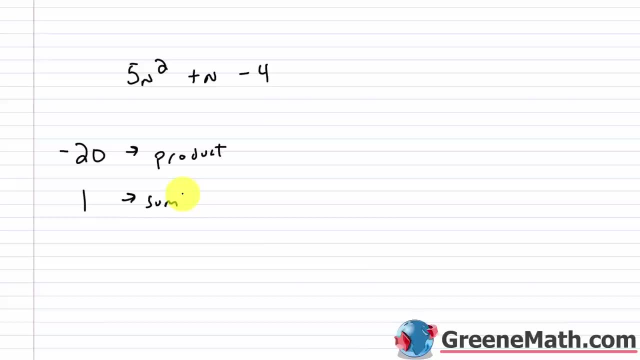 If I had positive 5 and negative 4, that would work out. So let's use those. 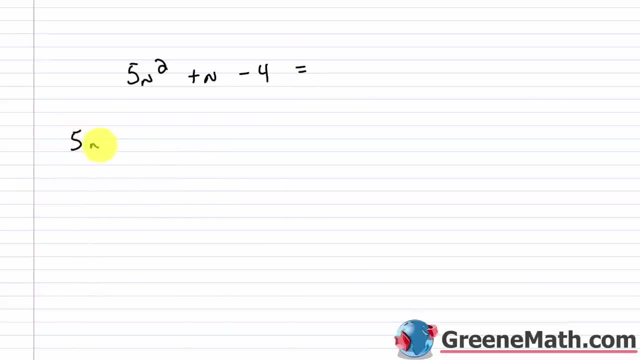 So we would have, this is equal to 5n squared plus 5n minus 4n minus 4. If we factor this by grouping, I could pull a 5n out of the first group. That would leave me with an n plus 1 here. Out of the second group, I can pull out a negative 4. That would leave me with n plus 1 here. So the common binomial factor is n plus 1. So I would have 5n minus 4, that quantity, times n plus 1, that quantity. So that's your factored form. All right, so let's erase this real quick. 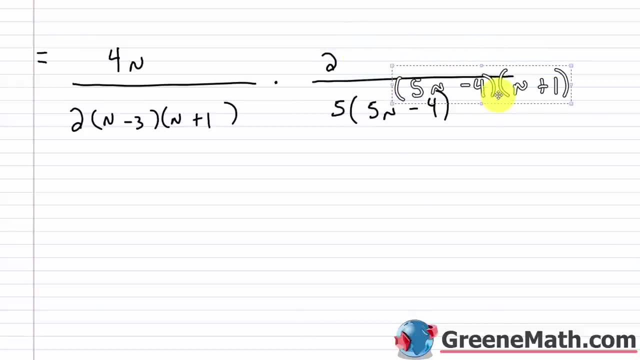 We'll put that factored form in here. Nice and convenient. 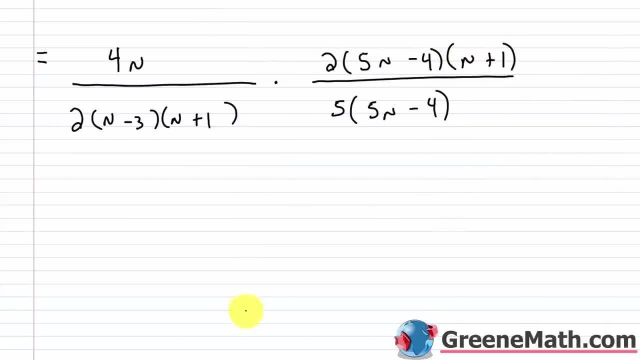 Okay, so now what we want to do is, we want to look to see what we can cancel. We have everything that's factored as much as we need to. And so I see that I have a common factor of 5n minus 4. Again, this is multiplication here. Everything is being multiplied. This is multiplication. So these are all factors. 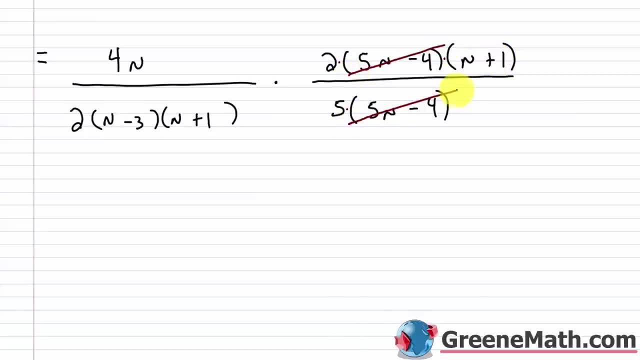 So this factor of 5n minus 4 will cancel with this factor of 5n minus 4. This factor of n plus 1 will cancel with this factor of n plus 1. We can cancel this 2 with this 2. And is there anything left? Nothing left that I can cancel. 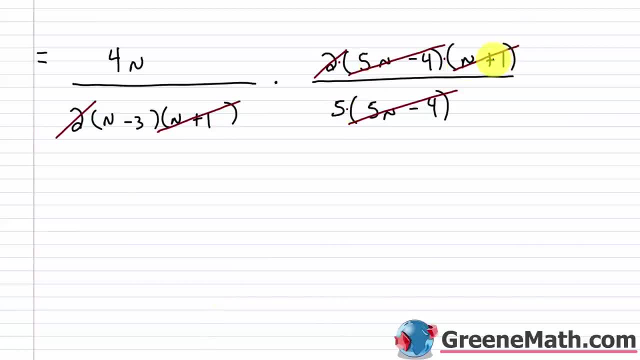 There's nothing up here other than a 1. Remember, when your numerator or your denominator cancels completely, you write a 1. 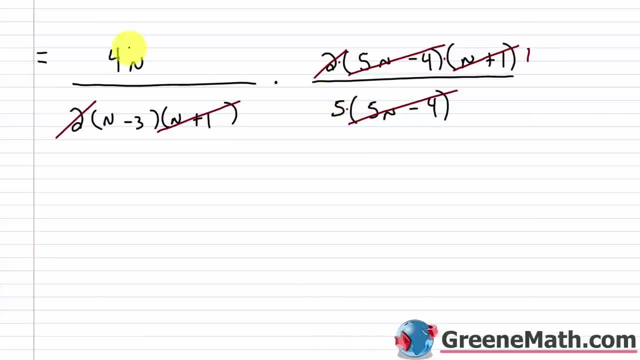 Down here, I just have a 5. So I need to be able to cancel a 5 with something over here I can't. So that's simplified. 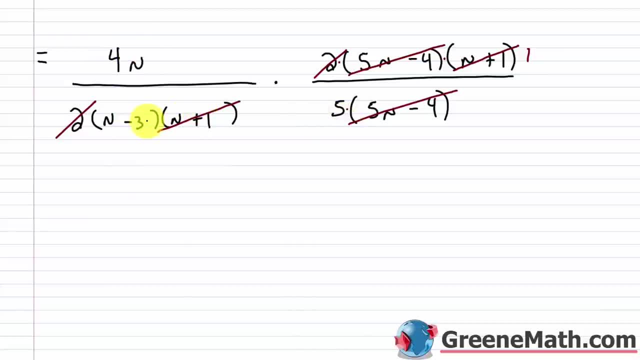 Over here, I have a 4n and I have an n minus 3. Nothing else I can do. 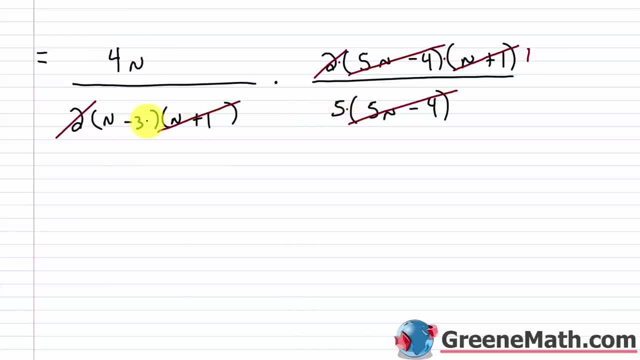 Over here. I have a 4n and I have a n minus 3.. Nothing else I can do. So when we multiply 4n times 1 is 4n. This is over. We have the quantity n minus 3 times 5.. 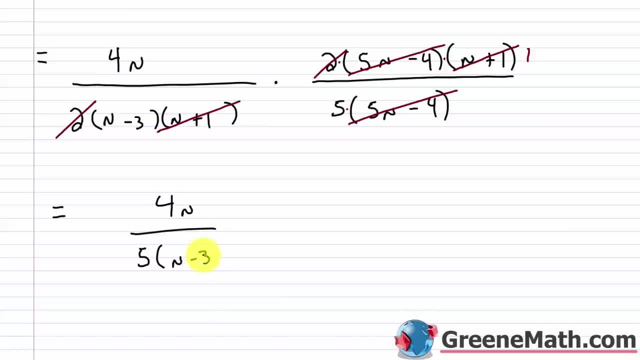 So we just write that as 5 times the quantity n minus 3.. Or you can leave it in this form, or you can write 4n over. Use your distributive property: 5n minus 5 times 3 is 15.. 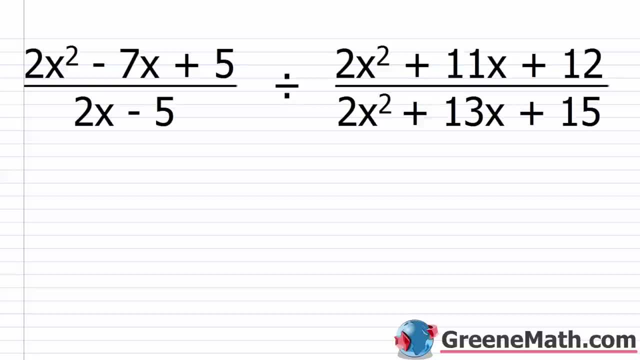 Okay, let's take a look at a null. So we have 2x squared minus 7x plus 5 over 2x minus 5.. This is divided by 2x squared plus 11x plus 12 over 2x squared plus 13x plus 15.. 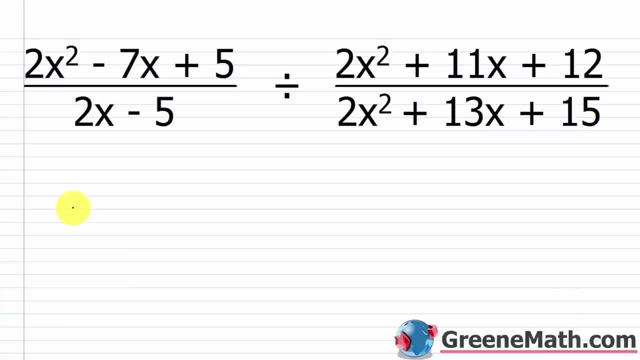 So for the first one in the numerator, 2x squared. 2x squared minus 7x plus 5. Let's see if we can factor that. So I would need two integers whose product is 10 and whose sum is negative 7. So let me start by just writing 2x squared. 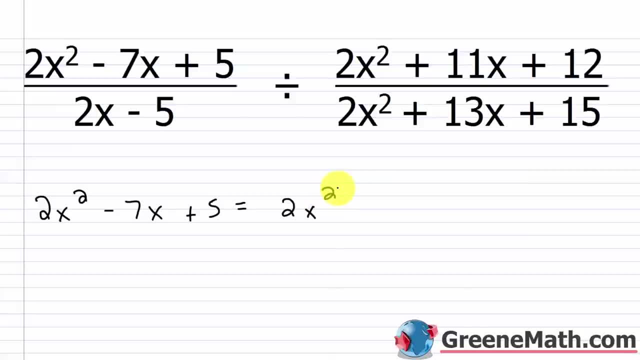 So if I think about the factors of 10, it's really 2 and 5.. If I did negative 5 and negative 2, that would work. So I would do minus 2x, then minus 5x, Then plus 5.. If I want to factor this by grouping, I'd pull out a 2x from the first group. 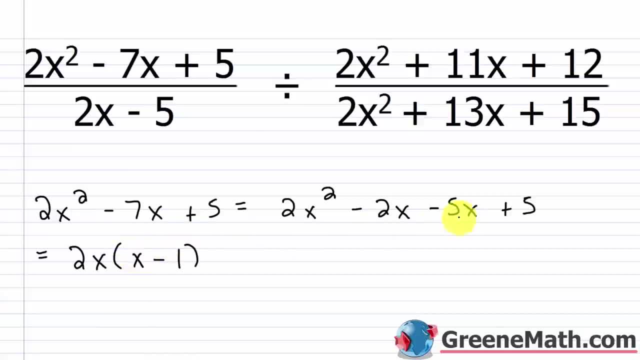 and I would have x minus 1.. From the second group I would pull out a negative 5. So minus 5 and that would give me an x minus 1.. And so if I pulled out the common binomial factor of x minus 1, 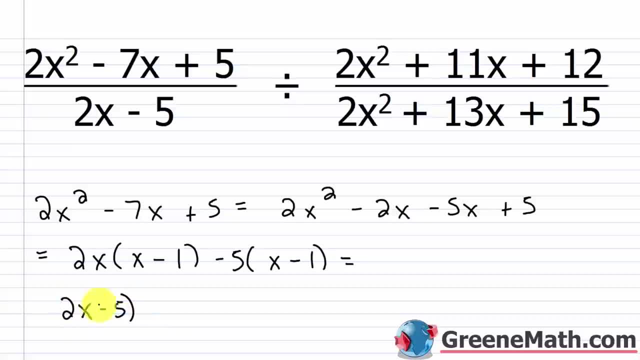 I would have 2x minus 5 times x minus 1.. All right, so let's erase all this And we'll kind of drag this up to the top. Put equals and we'll drag this up. Okay, so this is over 2x minus 5.. 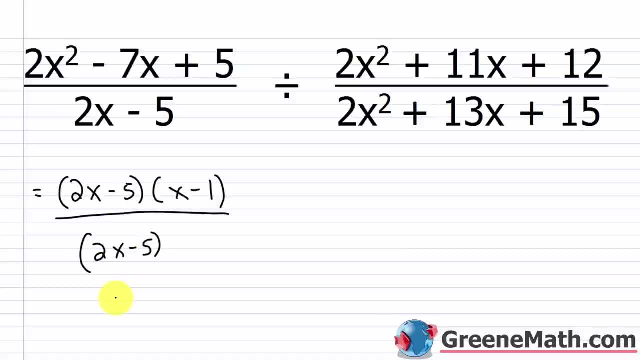 So we can cancel that right away if we want, or we can just kind of wait till we're done and we cancel everything at once. So that's what I'm going to do. Now. we're dividing by this guy right here, So let's just start by. 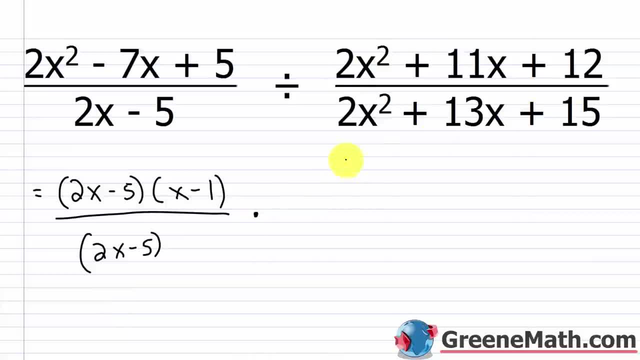 finding the reciprocal of x minus 5.. So let's just start by finding the reciprocal of x minus 5.. We're going to put multiplied by. I'm going to take the denominator here and put in the numerator 2x squared plus 13x plus 15.. And then, over the numerator, we'll go into the denominator. 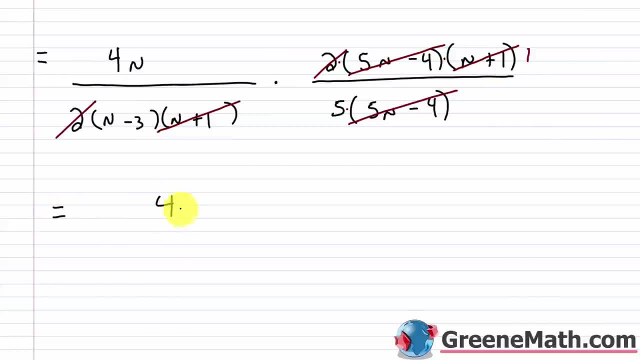 So when we multiply, 4n times 1 is 4n. This is over. We have the quantity n minus 3 times 5. So we just write that down. 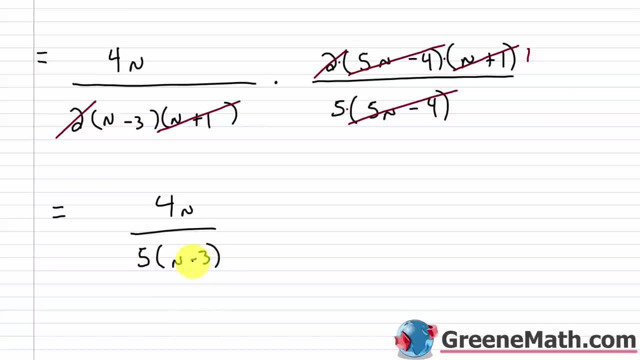 That is 5 times the quantity n minus 3. Or you can leave it in this form or you can write 4n over. 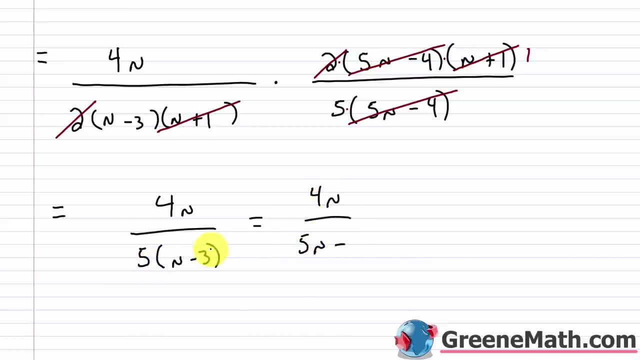 Use your distributive property, 5n minus 5 times 3 is 15. Okay, let's take a look at a null. 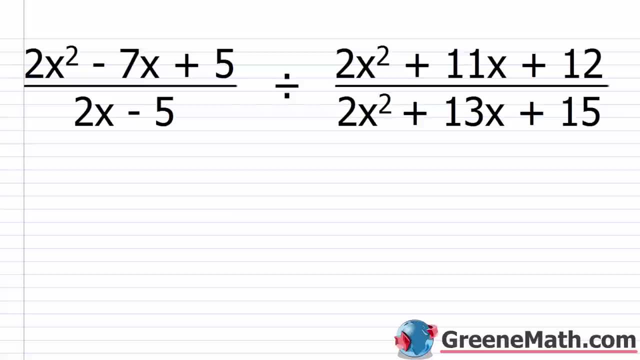 So we have 2x squared minus 7x plus 5 over 2x minus 5. This is divided by 2x squared plus 11x plus 12 over 2x squared plus 13x plus 15. So for the first one, in the numerator, 2x squared. 2x squared minus 7x plus 5. Let's see if we can factor that. 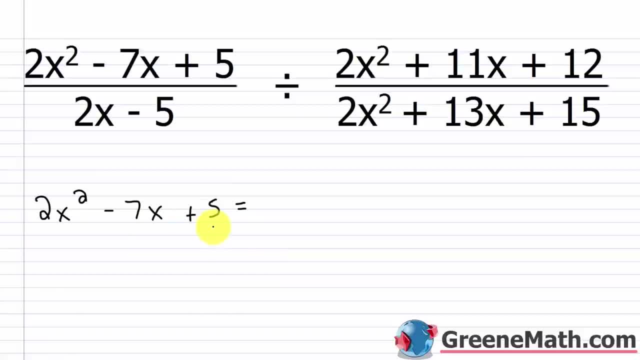 So I would need two integers whose product is 10 and whose sum is negative 7. So let me start by just writing 2x squared. 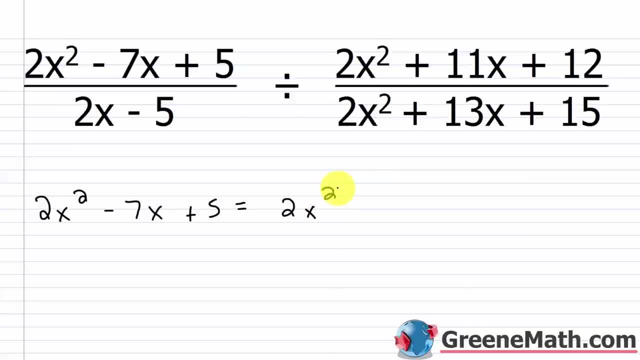 So if I think about the factors of 10, it's really 2 and 5. If I did negative 5 and negative 2, that would work. So I would do minus 2x then minus 5x. 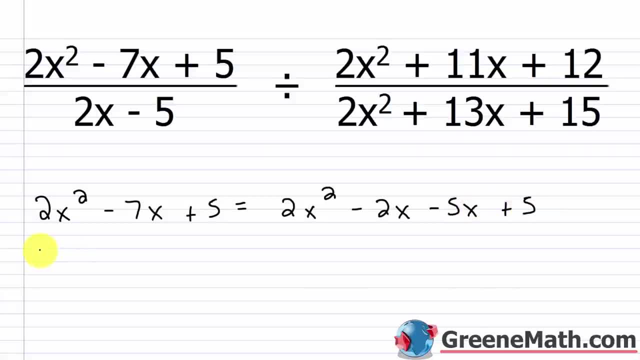 Then plus 5. If I want to factor this by grouping, I'd pull out a 2x from the first group. And I would have x minus 1. From the second group, I would pull out a negative 5. 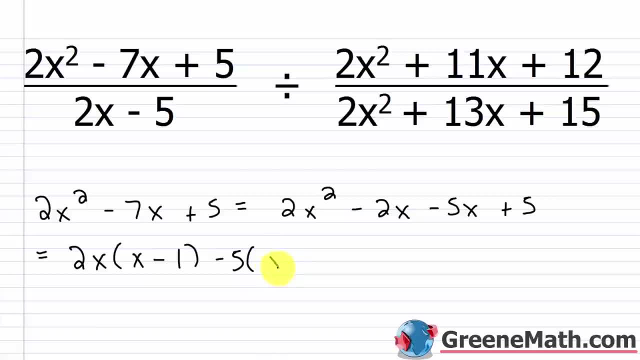 So minus 5. And that would give me an x minus 1. And so if I pulled out the common binomial factor of x minus 1, I would have 2x minus 5 times x minus 1. Alright, so let's erase all this. 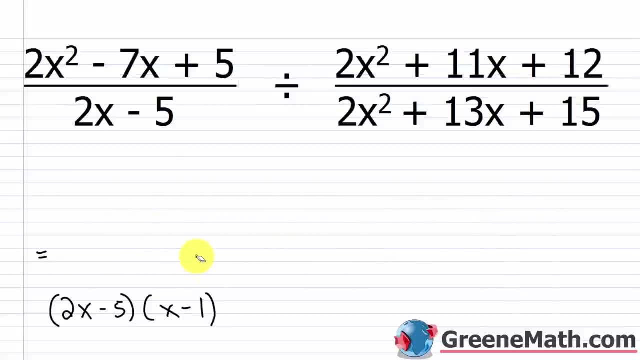 And we'll kind of drag this up to the top. Equals. And we'll drag this up. Okay, so this is over 2x minus 5. 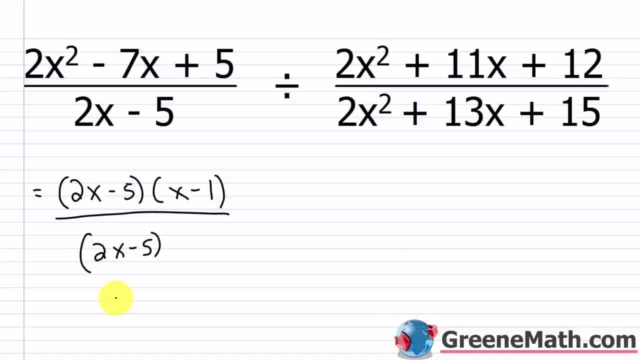 So we can cancel that right away if we want. Or we can just kind of wait until we're done. And we cancel everything at once. So that's what I'm going to do. 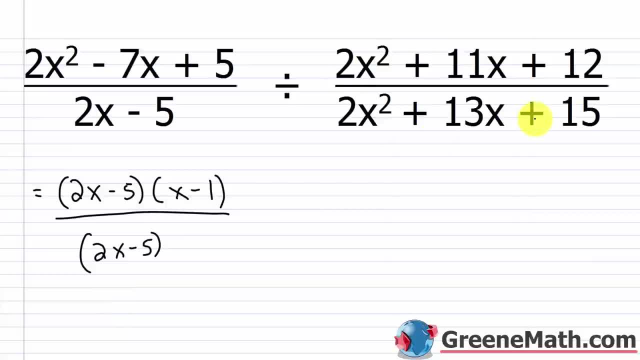 Now we're dividing by this guy right here. So let's just start by finding the reciprocal. We're going to put multiplied by. I'm going to take the denominator here and put it in the numerator. 2x squared plus 13x plus 15. And then over the numerator, we'll go into the denominator. 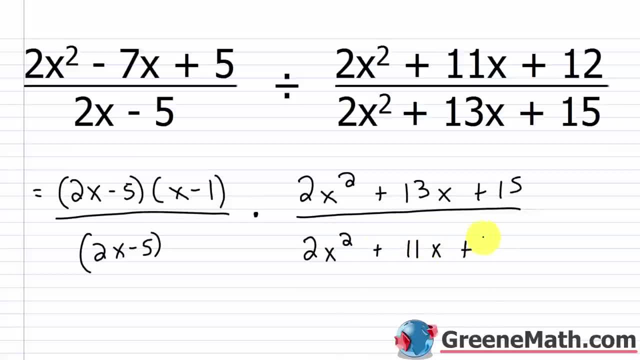 2x squared plus 11x plus 12. Okay. 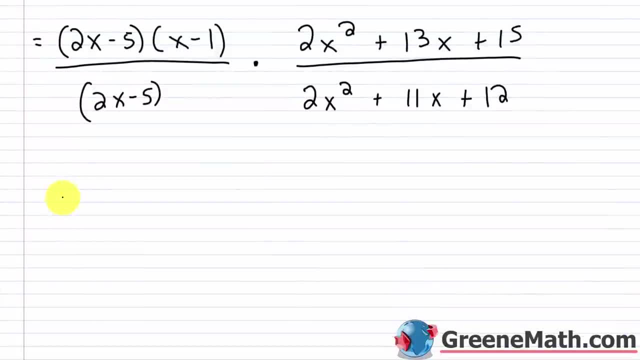 So let's factor each one separately here. So if I had 2x squared plus 13x plus 15. 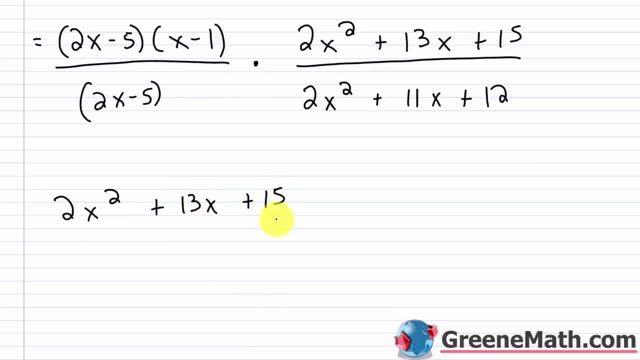 So two integers whose product is 30. And whose sum is 13. So for 30, I've got 1 times 30. I've got 2 times 15. Can I play with the signs there? 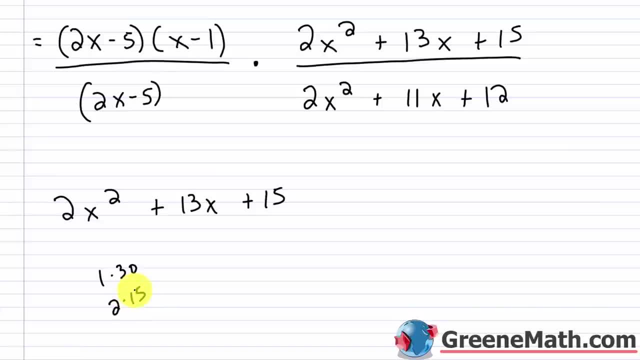 No, because everything is positive. So I can't really use that. 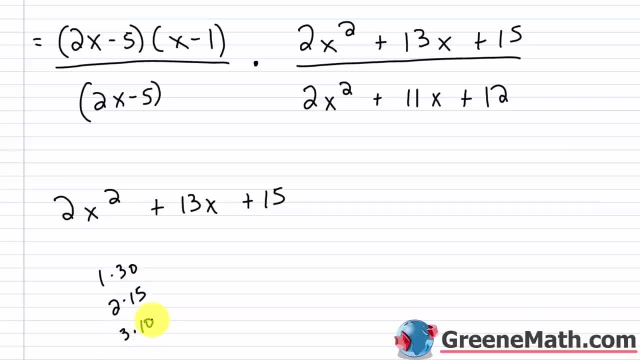 I've got 3 times 10. And that would work if I did positive 3 and positive 10. So let's go with that. 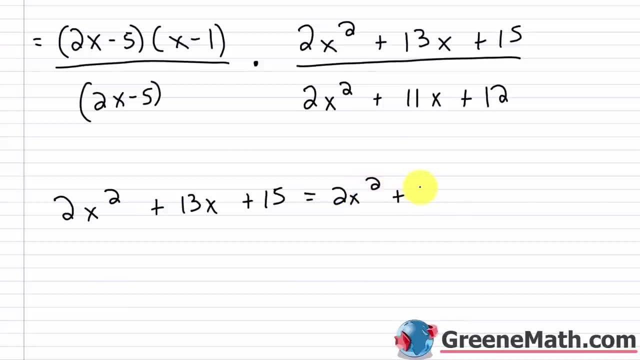 So then this equals 2x squared plus 10x plus 3x. Plus 15. And again, we're going to factor by grouping. 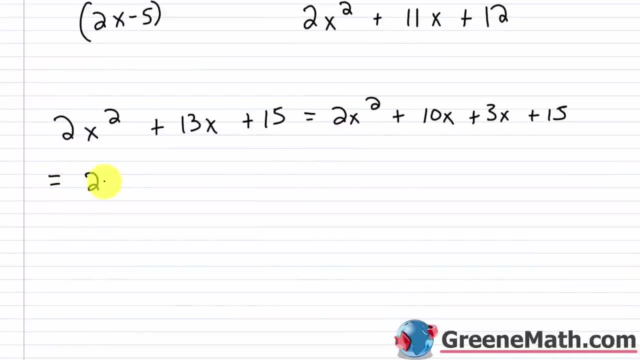 So from the first group, I'm going to pull out a 2x. That would leave me with an x plus 5. From the second group, I'll pull out a 3. That will leave me with x plus 5. And so pull out the common binomial factor of x plus 5. 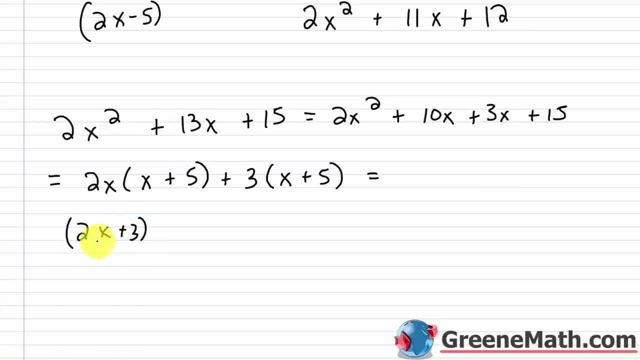 And you would get 2x plus 3. That quantity. Times x plus 5. That quantity. So let's copy this. All right. 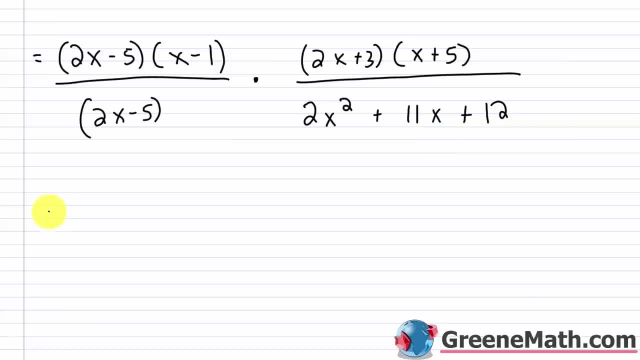 Let's also look at 2x squared plus 11x plus 12. So 2x squared plus 11x plus 12. 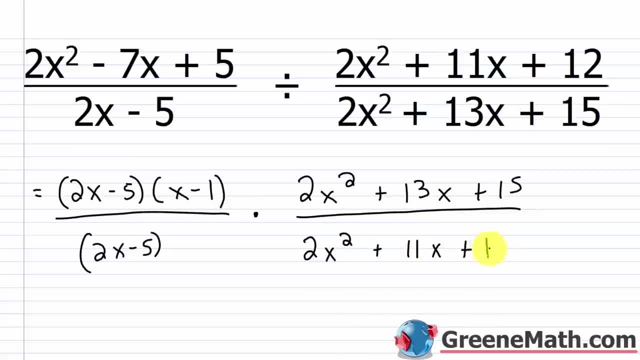 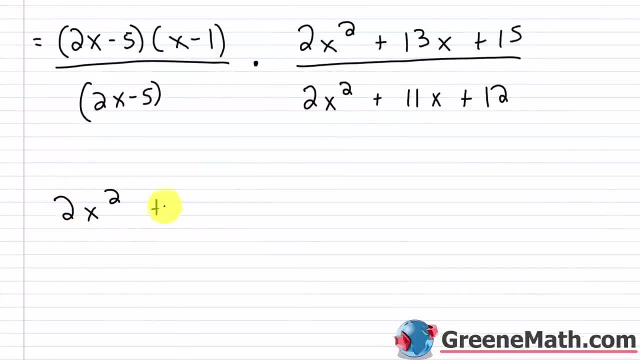 2x squared plus 11x plus 12.. Okay, so let's factor each one separately here. So if I had 2x squared plus 13x plus 15. So two integers whose product is 30 and whose sum is 13.. 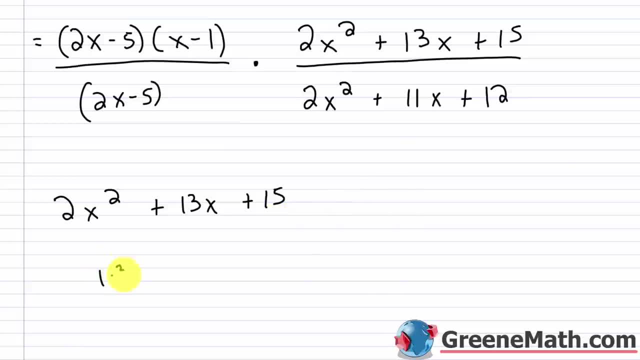 So for 30, I've got 1 times 30.. I've got 2 times 15.. Can I play with the signs there? No, because everything is positive right, So I can't really use that. I've got 3 times 10.. And that would. 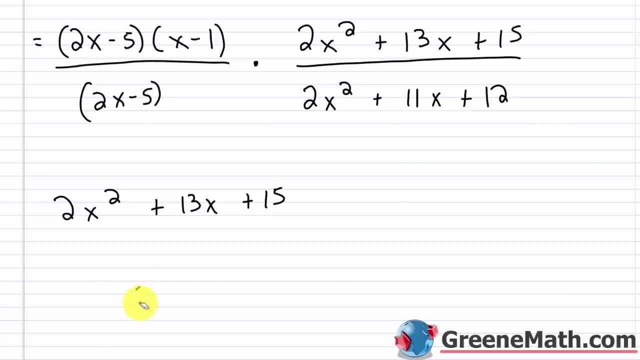 work if I did positive 3 and positive 10.. So let's go with that. So then this equals 2x squared plus 10x, plus 3x plus 15.. And again, we're going to do that. So let's go with that. So let's go with that. 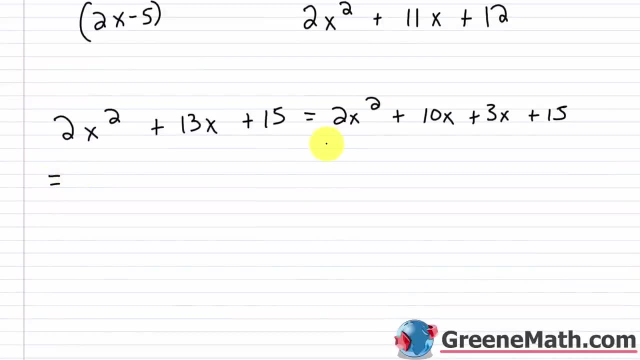 a factor by grouping. So from the first group, I'm going to pull out a 2x. That would leave me with an x plus 5.. From the second group, I'll pull out a 3.. That'll leave me with x plus 5.. And so pull out. 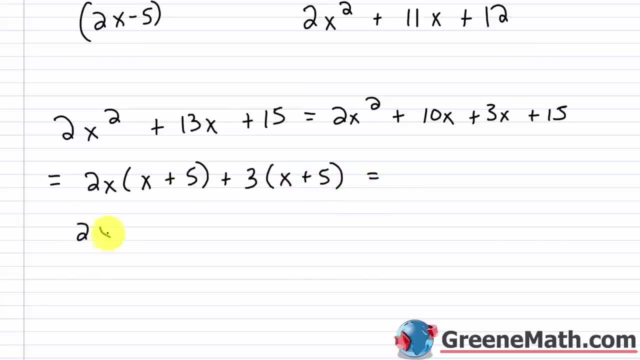 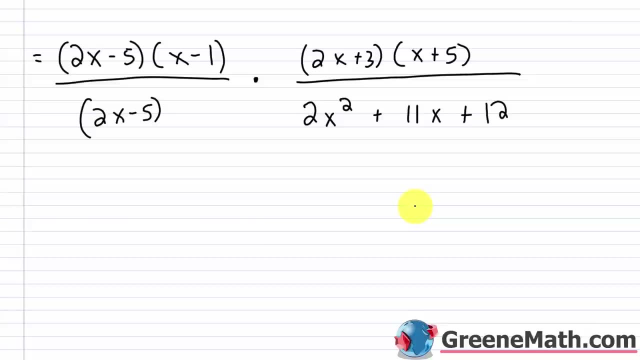 the common binomial factor of x plus 5. And you would get 2x plus 3. That quantity times x plus 5. That quantity, So let's copy this. All right. let's also look at 2x squared plus 11x plus 12.. 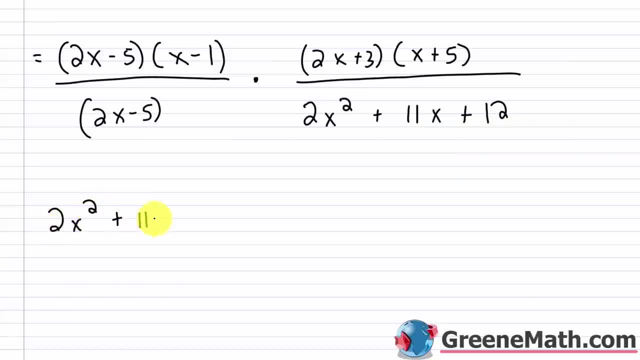 So 2x squared Plus 11x plus 12.. So for this, right here, let's think about two integers whose product is 24 and whose sum is 11.. So for 24, you do 1 times 24.. I can do 2 times 12.. I can do 3 times 8.. So 3 and. 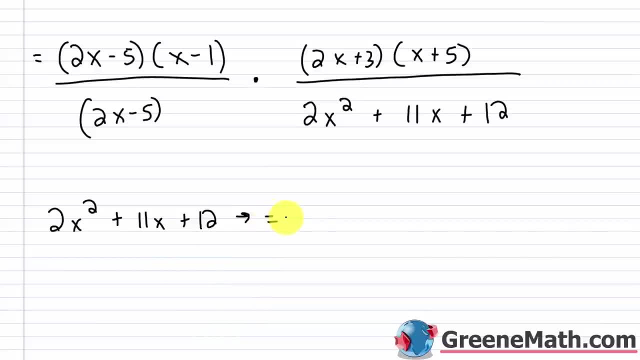 8 would work. So let's break this up. We'll say this equals 2x squared plus 8x plus 3x plus 12.. So in the first group I can pull out a 2x. So let's pull out 2x, And inside I would have what? 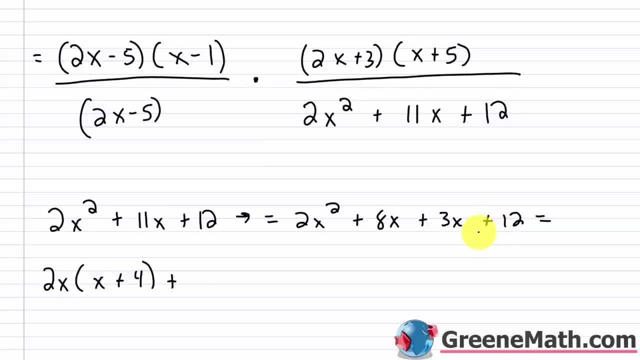 I would have x plus 4.. In the second group I can pull out a 3. So what I have left is again x plus 4. So the common binomial factor here is x plus 4.. So let's go ahead and pull that guy out and I. 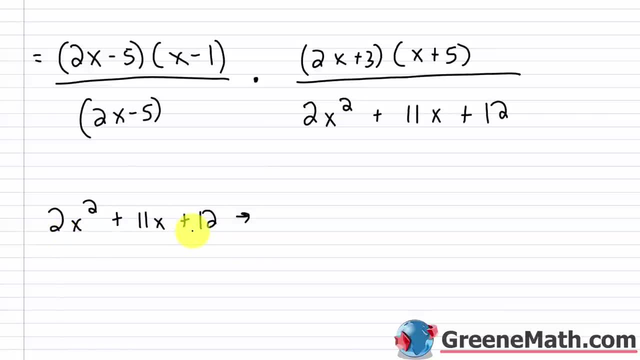 So for this right here, let's think about two integers whose product is 24 and whose sum is 11. So for 24, you do 1 times 24. I can do 2 times 12. I can do 3 times 8. So 3 and 8 would work. So let's break this up. 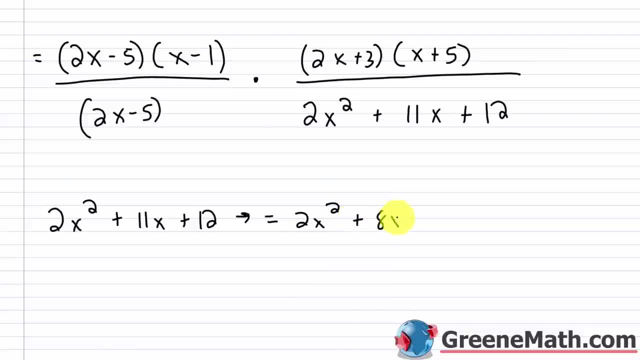 We'll say this equals 2x squared. Plus 8x plus 3x plus 12. 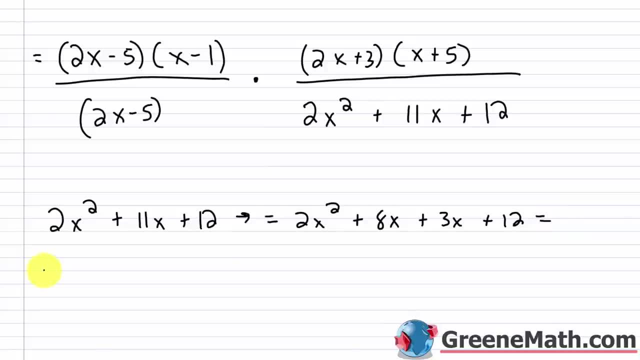 So in the first group, I can pull out a 2x. So let's pull out 2x. And inside, I would have what? I would have x plus 4. In the second group, I can pull out a 3. So what I have left is, again, x plus 4. 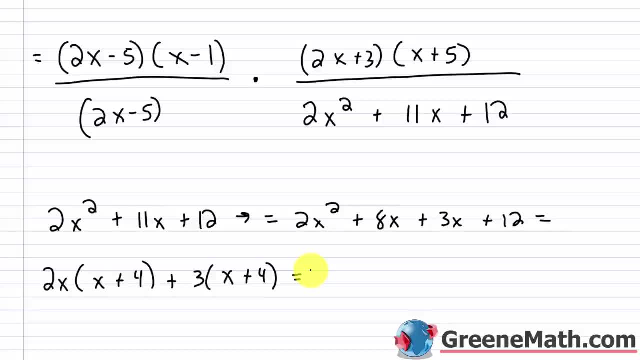 So the common binomial factor here is x plus 4. So let's go ahead and pull that guy out. And I have 2x plus 3. Times. Times x plus 4. 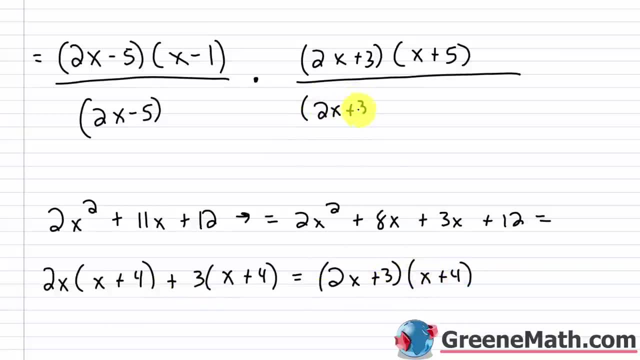 So this is 2x plus 3 times x plus 4. 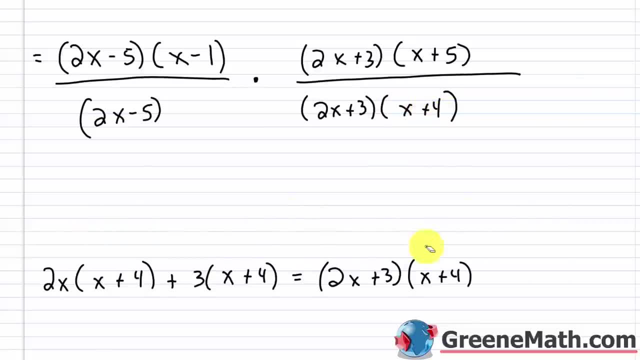 So now that we've factored everything, I know that's the kind of tedious, boring part. But once you've gotten through that, the rest of it's pretty simple. I'm just going to look for common factors and cancel. 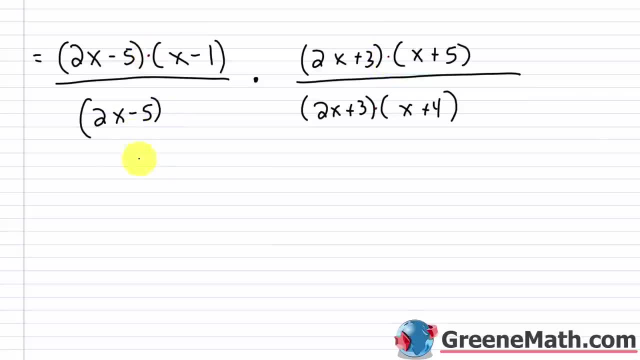 Remember, everything is being multiplied. So these are common factors. So I can put this as times 1 here. And I can cancel 2x minus 5. That factor with 2x minus 5 up here. And then I don't have any x minus 1s anywhere else. I can't do anything with that. But I can cancel this factor of 2x plus 3 with this factor of 2x plus 3. And what I'm left with is x minus 1. 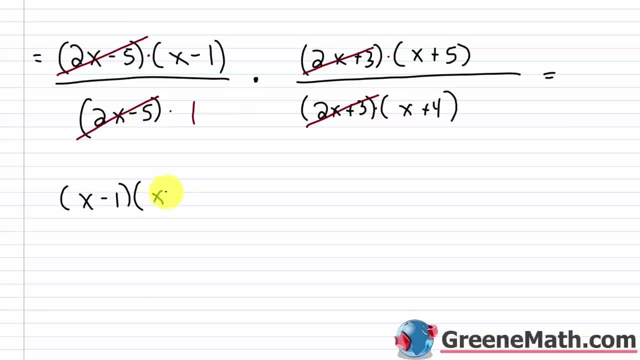 So x minus 1. And times x plus 5. Over 1 times x plus 4. 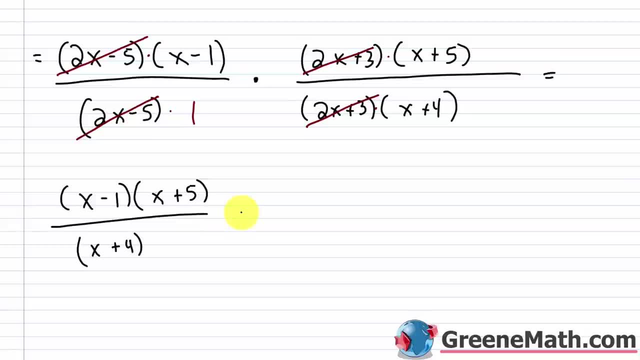 So basically x plus 4. Now, you can leave it in this format if you want. 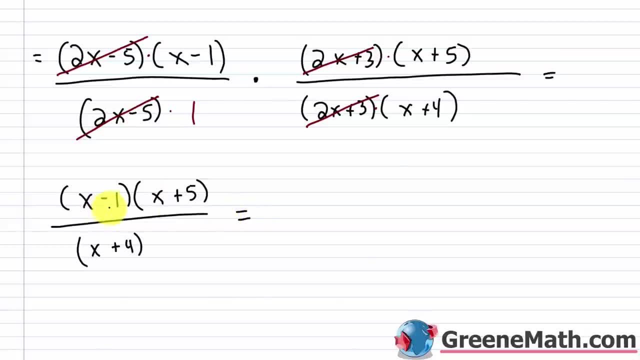 Or your teacher might want you to use FOIL and present this as a trinomial in the top. That's fine. Either way, it's the same thing. 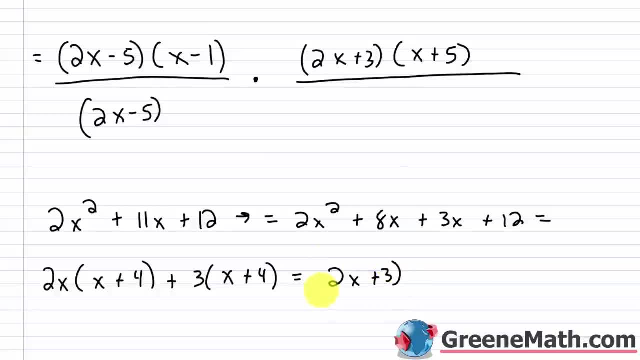 have 2x plus 3, times x plus 4.. So this is 2x plus 3.. Times x plus 4.. So now that we've factored everything- I know that's the kind of tedious, boring part, But once you've gotten through that, the rest of it's pretty simple. I'm just going to. 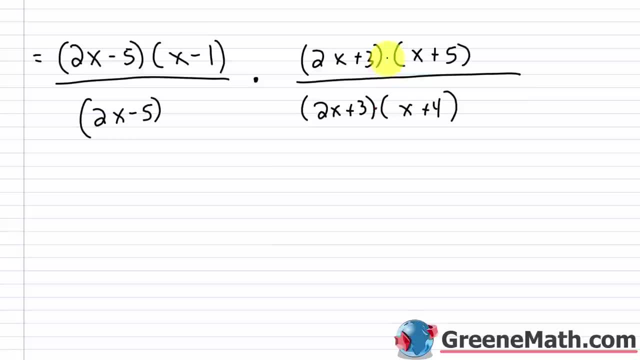 look for common factors and cancel. Remember, everything is being multiplied, So these are common factors. So I can put this as times 1 here And I can cancel 2x minus 5.. That factor with 2x minus 5 up here, And then I don't have any x minus 1s anywhere else. I can't do anything. 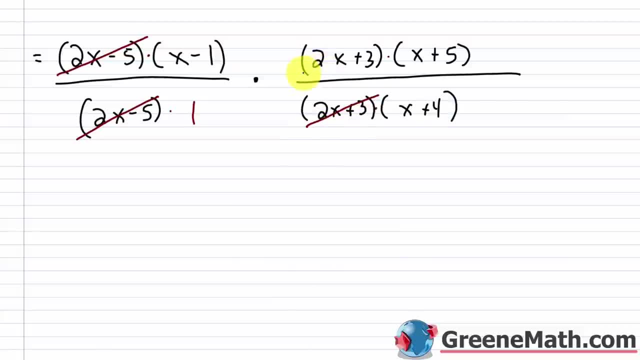 with that, I can cancel this factor of 2x plus 3 with this factor of 2x plus 3.. And what I'm left with is x minus 1.. So x minus 1.. And times x plus 5 over 1, times x plus 4.. So basically x plus 4.. Now you can. 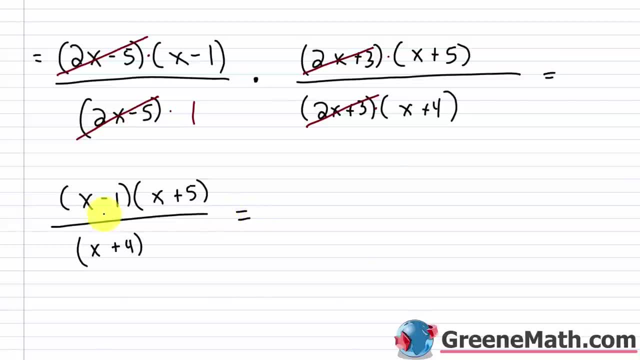 leave it in this format. if you want, Or your teacher might want you to use FOIL and present this as a trinomial in the top, That's fine. Either way it's the same thing. So x times x is x squared, The outer would be 5x, The inner would be minus x. So this is plus 4x And then the final. 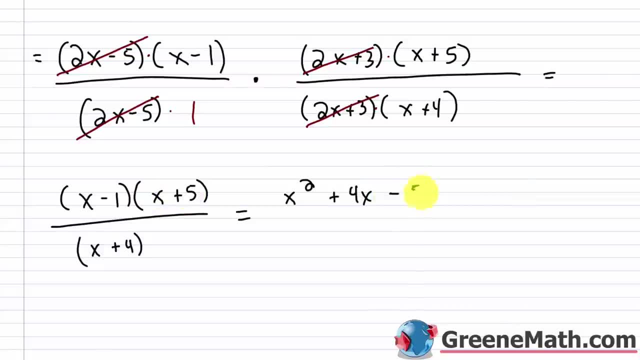 or the last would be negative 1 times 5, which is minus 5.. And again, this is over x plus 4.. So you get x squared plus 4x minus 5 over x plus 4.. All right, let's take a look at one final problem. 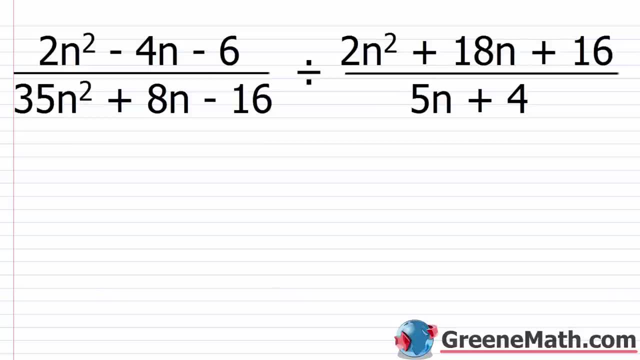 So I have 2n squared minus 4n minus 6.. This is over 35n squared plus 8n minus 16.. This is divided by x squared plus 4n minus 6.. This is over 35n squared plus 8n minus 16.. This is divided by: 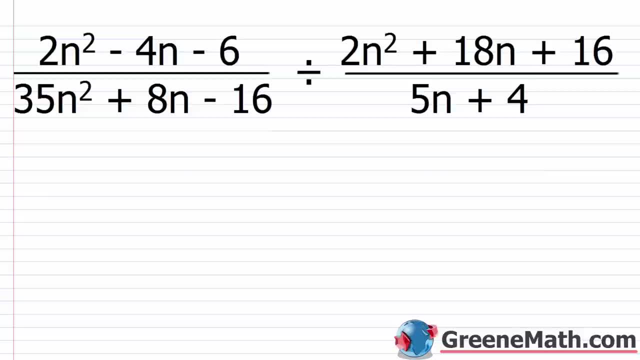 2n squared plus 18n plus 16 over 5n plus 4.. So I want to just factor everything here and see what's going to cancel. So if I start out in the numerator, I have 2n squared minus 4n minus 6.. 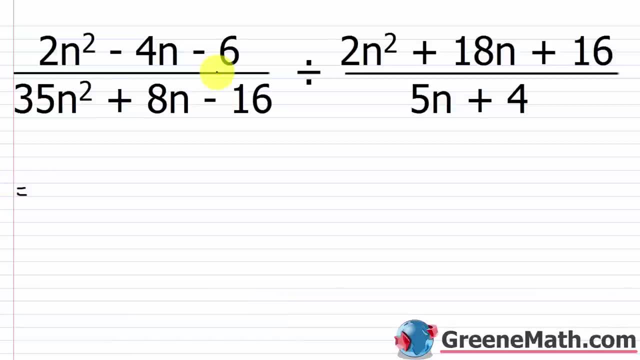 And in this particular case we've already factored this in a previous problem. So I'd pull a 2 out to start, And what I'd have is I'd have n squared minus 2n minus 3.. So give me two integers whose. So x times x is x squared. 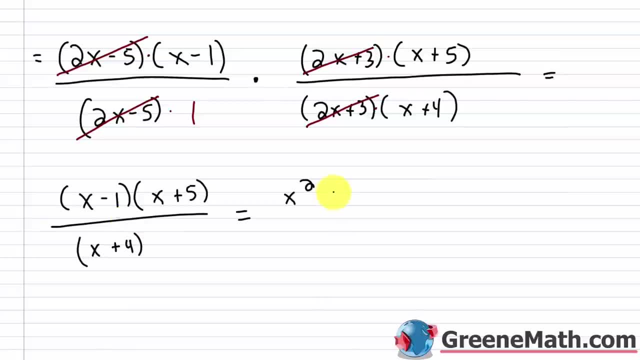 The outer would be 5x. The inner would be minus x. So this is plus 4x. And then the final, or the last, would be negative 1 times 5, which is minus 5. And again, this is over x plus 4. So you get x squared plus 4x minus 5 over x plus 4. 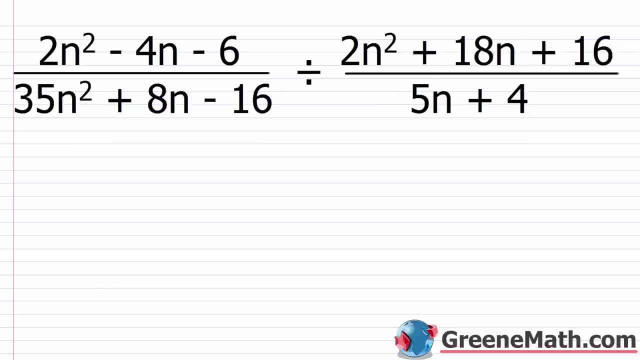 Alright, let's take a look at one final problem. So I have 2n squared minus 4n minus 6. 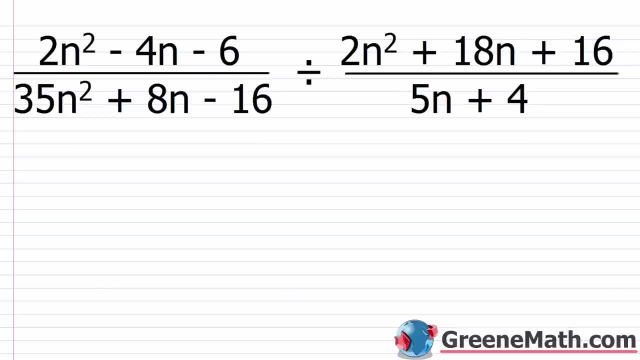 This is over 35n squared plus 8n minus 16. 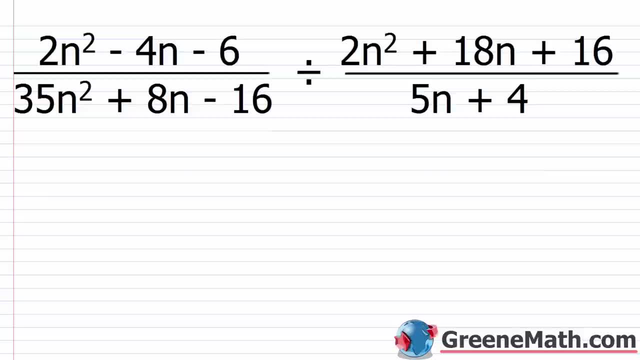 This is divided by 2n squared plus 18n plus 16 over 5n plus 4. So I want to just factor everything here and see what's going to cancel. 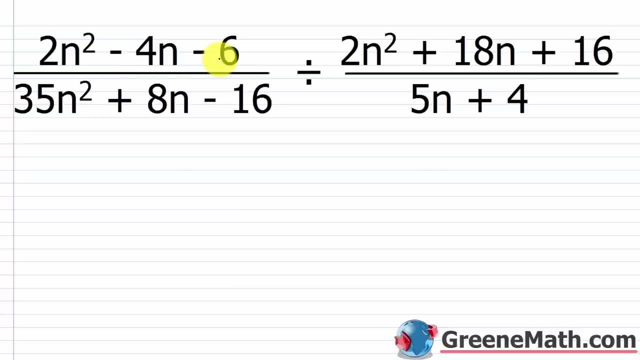 So if I start out in the numerator, I have 2n squared minus 4n minus 6. And in this particular case, we've already factored this in a previous problem. So I'd pull a 2 out to start. And what I'd have is, I'd have n squared minus 2n minus 3. So give me two integers whose product is negative 3 and whose sum is negative 2. Well, that would be negative 3 and positive 1. So I would have n minus 3, n minus 3, and then n plus 1. And a lot of you will remember that again from a previous problem. 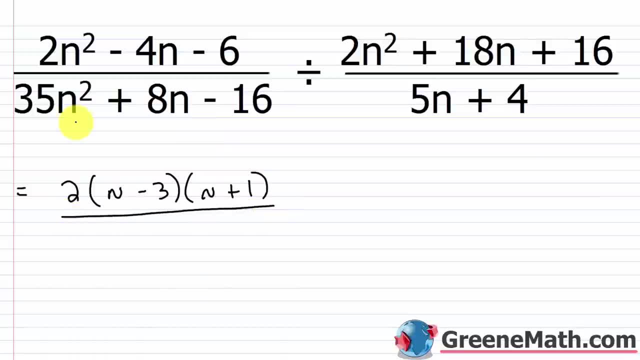 So this is going to be over. I need to factor that down here because I'm going to need a little room to do that. 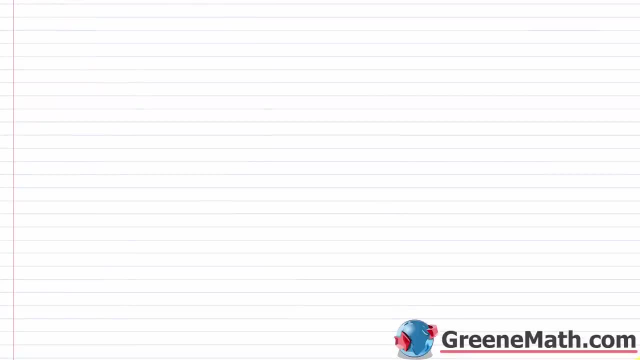 So let's kind of scroll down a little bit. So 35n squared plus 8n minus 16. 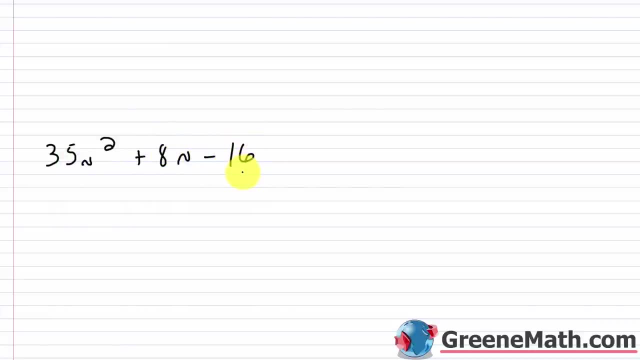 So if I multiply 35 times negative 16, I would get negative 560. And that's what I'm looking for as far as the product. 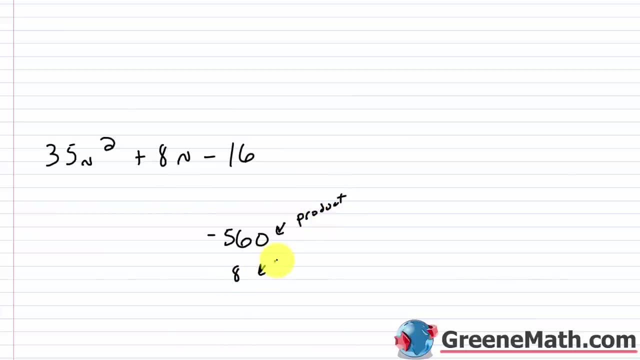 For my sum, I want 8. Now, most of us do not work with numbers. 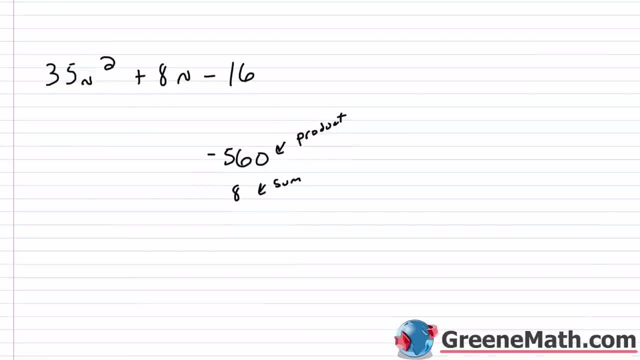 We work with 560 a lot. So this is something to where you want to make a factor tree and kind of think about what the prime factorization is. 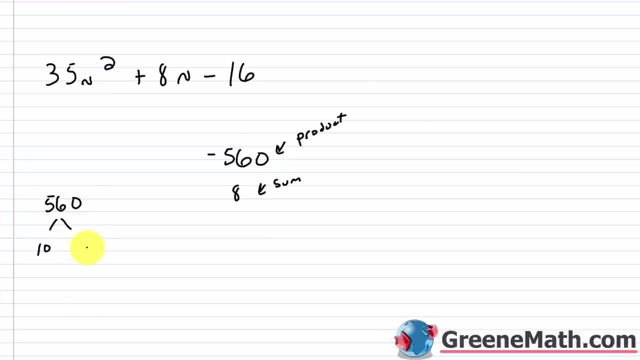 So I would just start with something like, you know, 10 times 56. Nice and simple. 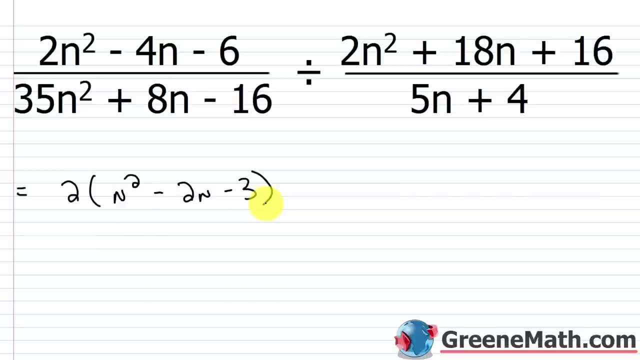 product is negative 3 and whose sum is negative 2.. Well, that would be negative 3 and positive 1.. So I would have n minus 3, n minus 3 and then n plus 1.. And a lot of you will remember that again. 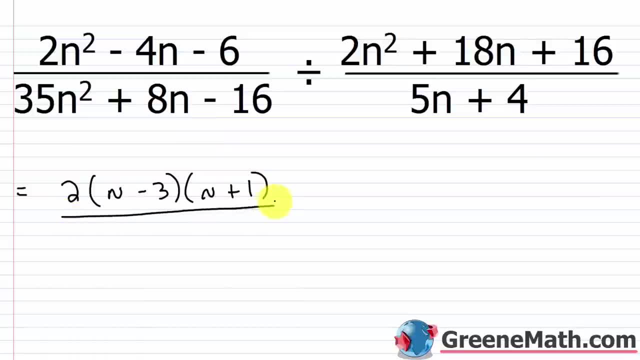 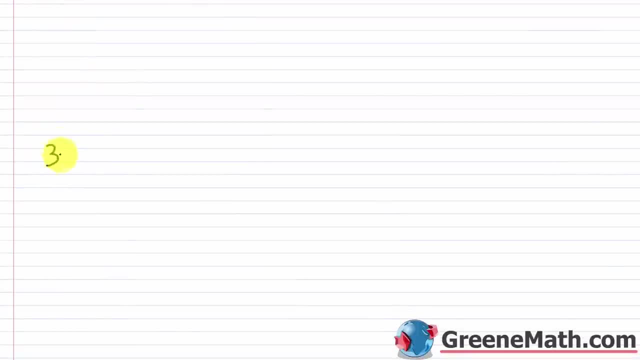 from a previous problem. So this is going to be over. I need to factor that down here because I'm going to need a little room to do that. So let's. let's kind of scroll down a little bit. So 35n squared plus 8n. 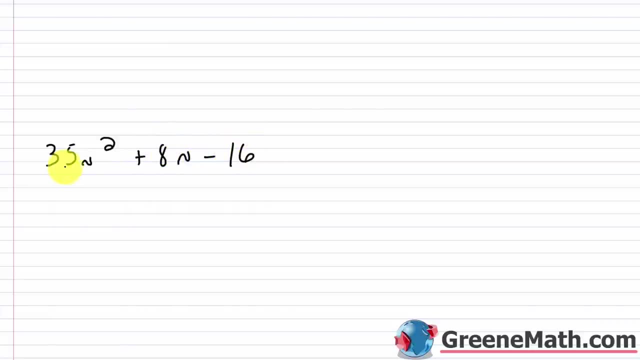 Minus 16.. So if I multiply 35 times negative 16, I would get negative 560. And that's what I'm looking for as far as the product. For my sum I want 8.. Now, most of us do not work with 560 a lot, So this is something to where you want to make a factor. 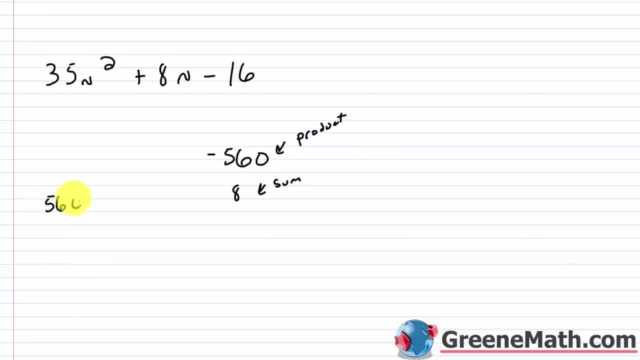 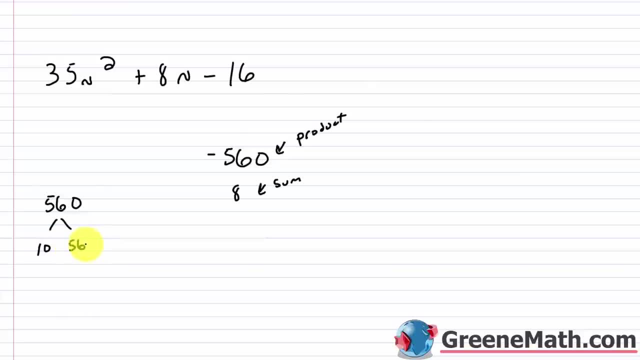 If I did 10 times 56. Okay, nice and simple. So that's obviously not close for me. So then, 10 is 5 times 2.. 56 if I did 28 times 2.. Now I want you to notice something here. 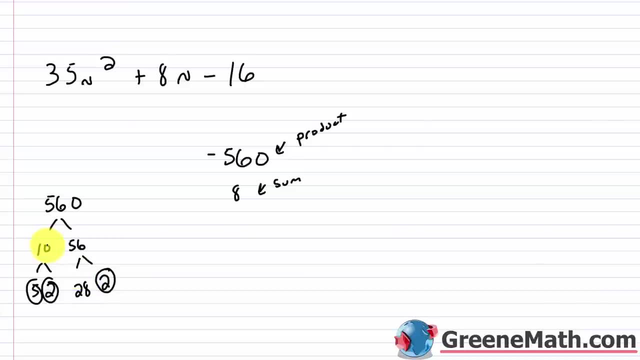 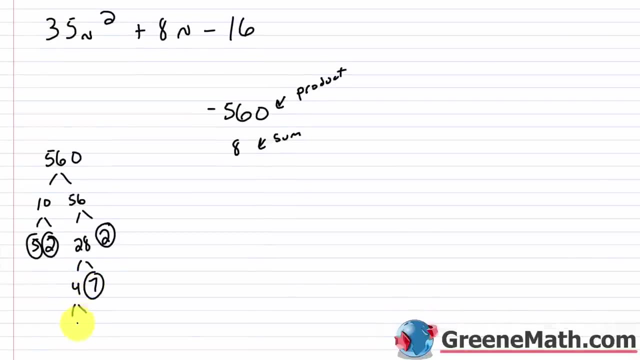 If I have 28 times 20.. 28 and 20- I can make that work. So I could stop here. For the sake of the factor tree, let's just continue. This is 4 times 7.. And then 4 is 2 times 2.. And then 4 is 2 times 2.. 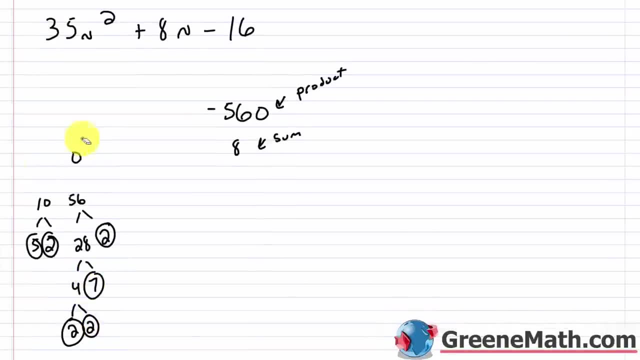 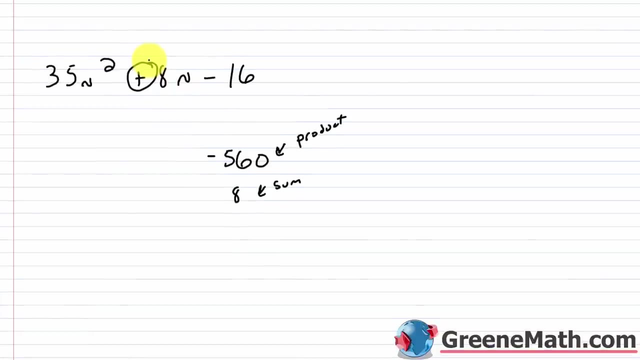 times 2. so let me kind of erase this. now we have our two integers, so we know it's 20 and 28. what do the signs need to be? well, since the sum is positive, I want the larger absolute value to be positive. so I want to do positive 28 and negative 20. so let's erase this real quick. let's say okay. 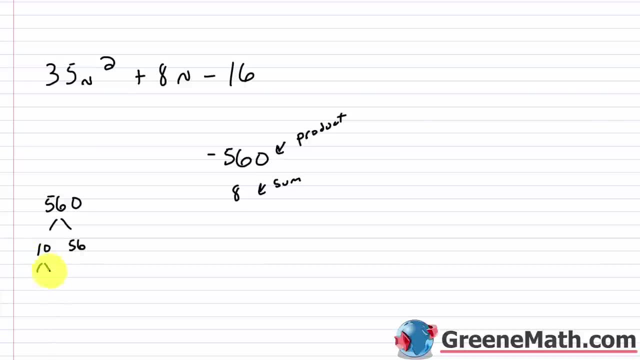 So that's obviously not close for me. So then 10 is 5 times 2. 56, if I did 28 times 2. Now, I want you to notice something here. If I have 28 times 20, 28 and 20, I can make that work. So I could stop here. For the sake of the factor tree, let's just continue. 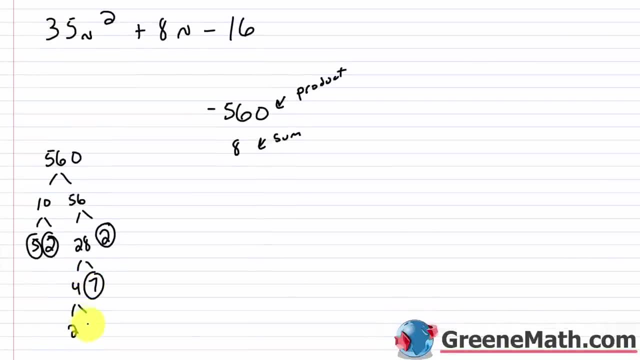 This is 4 times 7. And then 4 is 2 times 2. So let me kind of erase this now. We have our two integers. So we know it's 20 and 28. 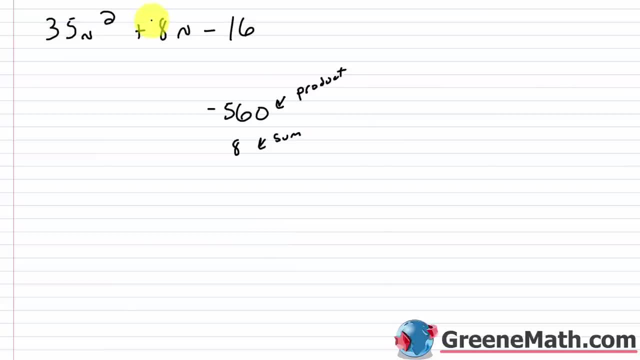 What do the signs need to be? Well, since the sum is positive, I want the larger absolute value to be positive. So I want to do positive 28 and negative 20. So let's erase this real quick. 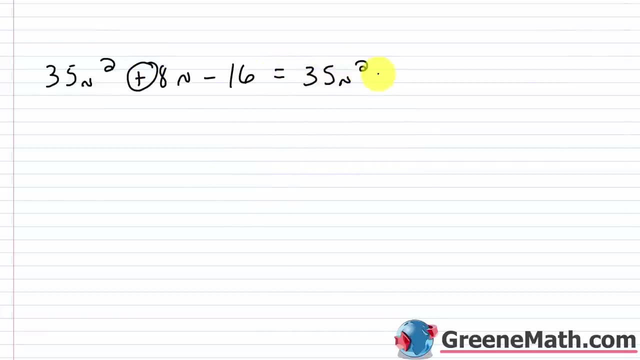 Let's say, OK, we have 35n squared plus 28n minus 20n and then minus 16. OK. 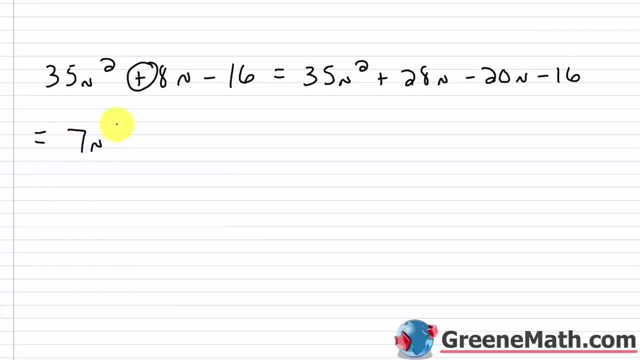 So in the first group, I could pull out a 7n. So this would be 7n. And what would be left is 5n plus a 4. In the second group, I can pull out a negative 4. And what would be left would be 5n. 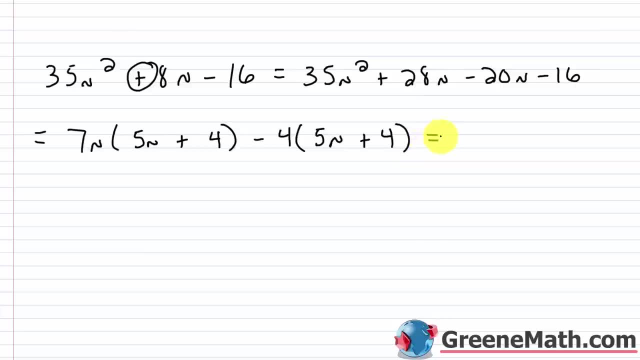 Plus 4. So if I factor out the common binomial factor of 5n plus 4, I would have 7n minus 4 times 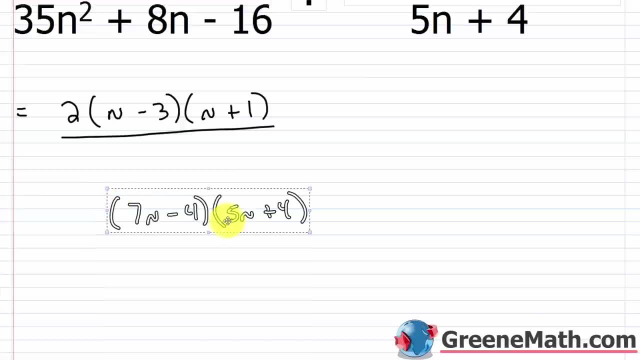 So let's go ahead and copy this. OK. We're going to paste this right here. OK. Now, the rest of this is pretty simple. Now, we're dividing by. 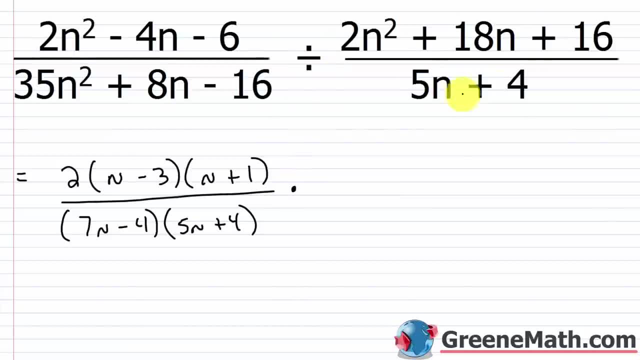 So I'm going to put a multiplication sign here. And then I'm going to take the reciprocal of this. So the 5n plus 4 is going to go up top. 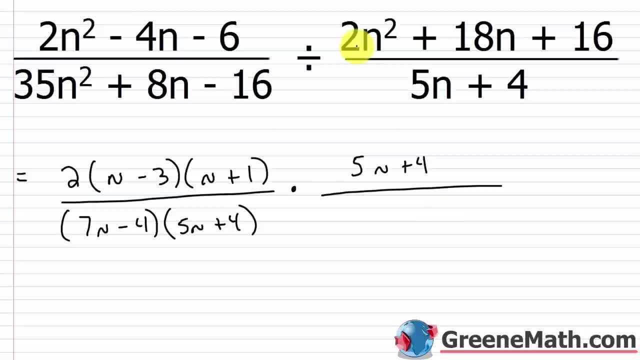 In the denominator here, I can factor out a 2 before I start. So that's going to make things simpler. 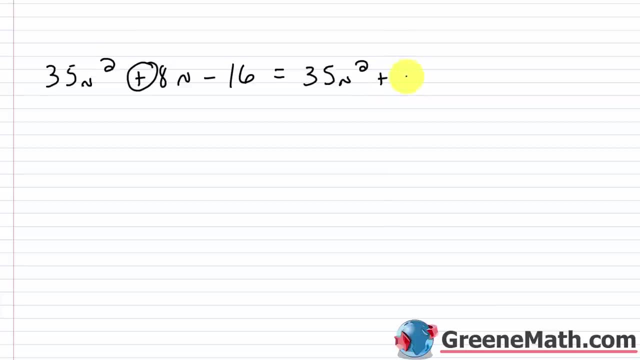 we have 35n squared plus 28n, minus 20n and then minus 16. okay, so in the first group I could pull out a 7n, so this would be 7n and what would be left is 5n plus a 4. in the second group, I can. 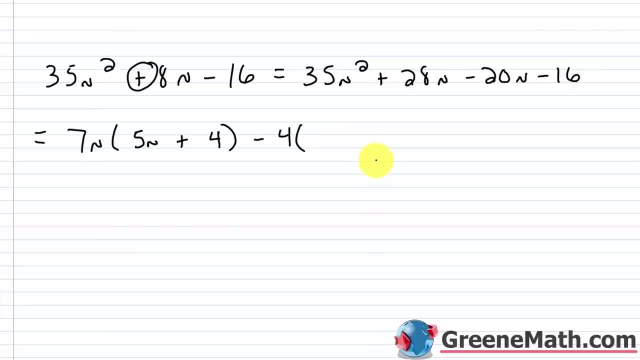 pull out a negative 4 and what would be left would be 5n plus 4. so if I could pull out a negative 4 and what would be left would be 5n plus 4, I factor out the common binomial factor of 5n plus 4, I would have 7n minus 4 times 5n plus 4.. 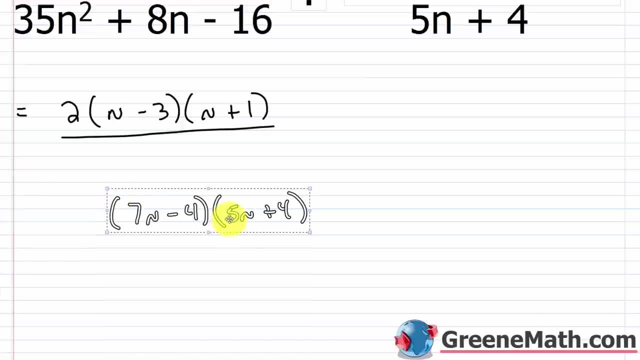 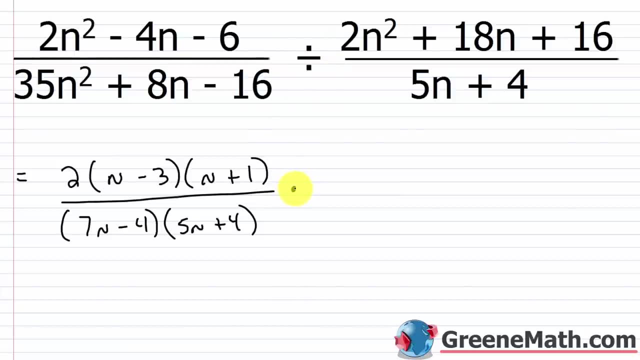 Let's go ahead and copy this. Okay, we're going to paste this right here. Okay, now the rest of this is pretty simple. Now we're dividing by. so I'm going to put a multiplication sign here And then I'm going to take the reciprocal of this, So the 5n plus 4 is going to go up top. 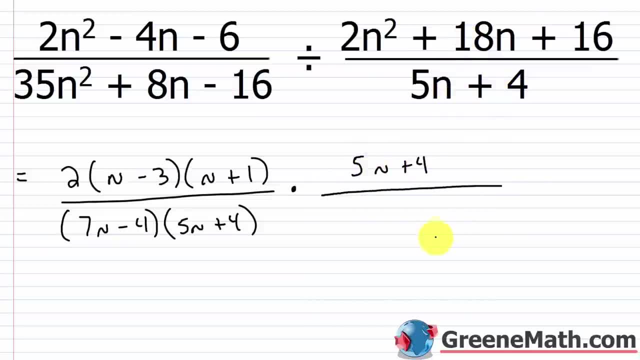 And the denominator. here I can factor out a 2 before I start. So it's going to make things simpler, And I'd have n squared plus 9n plus 8.. Now give me two integers, whose sum is 9 and whose product is 8.. Well, that would just be 8 and 1. So we would do n plus 8. 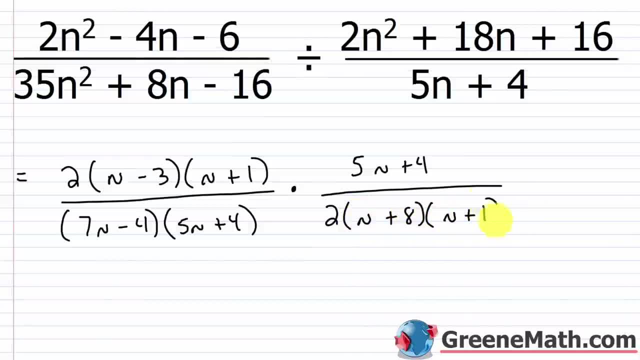 and then n plus 1.. Now I've got this as factored as I can get it. All I want to do now is look to see what I can cancel. So I can cancel a common factor of n plus 1.. I can cancel a common factor of 5n plus 4.. Remember, I could write this as times 1.. 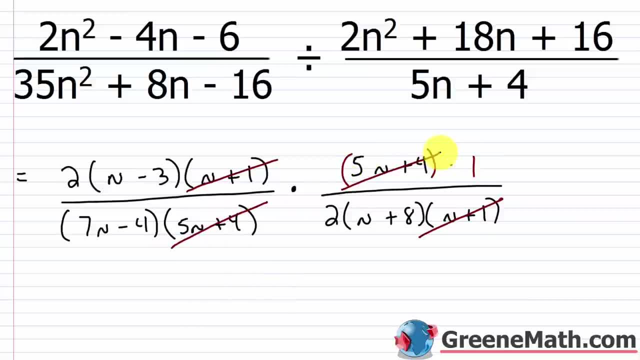 So this would cancel with this And then anything else I can cancel. I can cancel this 2 with this 2.. And what I'm looking at in my numerator, I'm going to have an n minus 3. In my denominator. 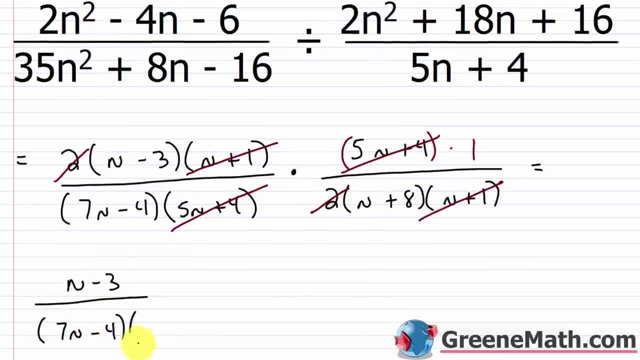 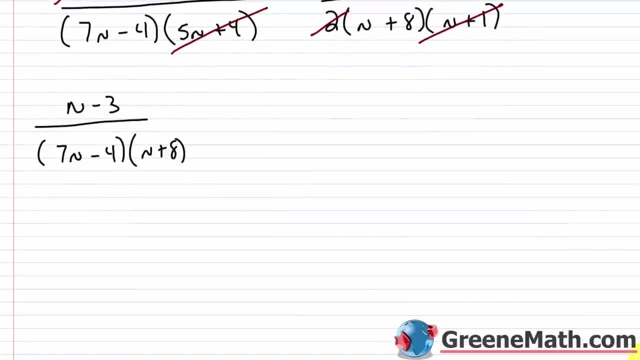 I'll have this quantity 7n minus 4 times this quantity n plus 8.. Now again, in a lot of cases you can just write this and stop. Your teacher might not want you to kind of come down here in the denominator and do FOIL, but she might want you to do it. It doesn't matter, It's the. 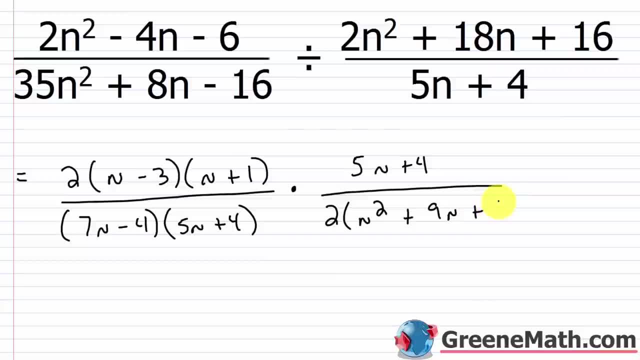 And I'd have n squared plus 9n plus 8. Now, give me two integers whose sum is 9 and whose product is 8. Well, that would just be 8 and 1. So we would do n plus 8 and then n plus 1. 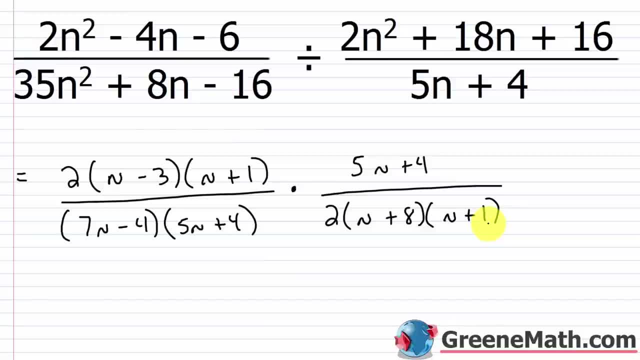 Now, I've got this as factored as I can get it. All I want to do now is look to see what I can get. So I can cancel a common factor of n plus 1. I can cancel a common factor of 5n plus 4. Remember, I could write this as times 1. So this would cancel with this. And then anything else I can cancel. I can cancel this 2 with this 2. And what I'm looking at in my numerator, I'm going to have an n minus 3. 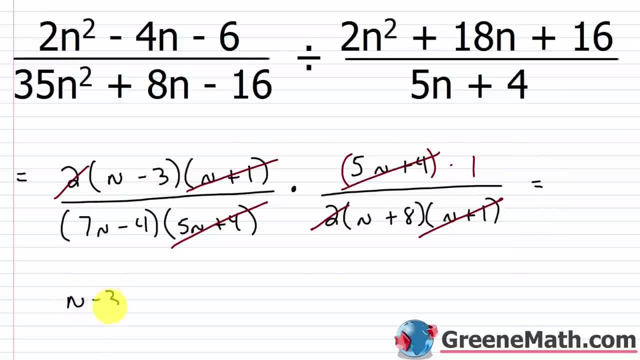 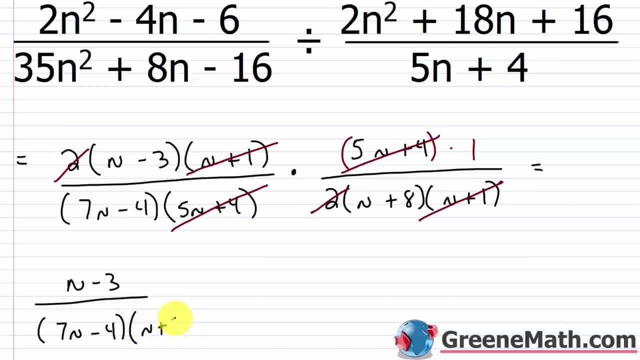 In my denominator, I'll have this quantity 7n minus 4. And I'm going to write this as times 1. 7n minus 4 times this quantity n plus 8. 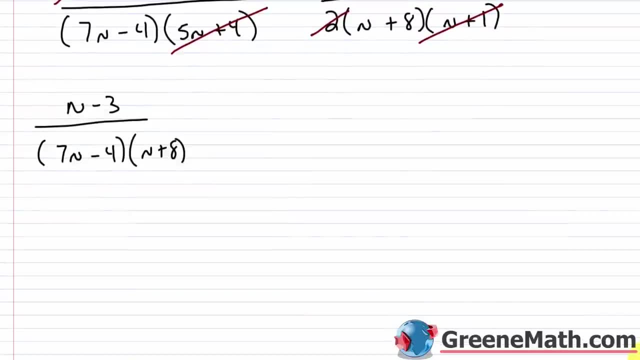 Now, again, in a lot of cases, you can just write this and stop. Your teacher might not want you to kind of come down here in the denominator and do FOIL. 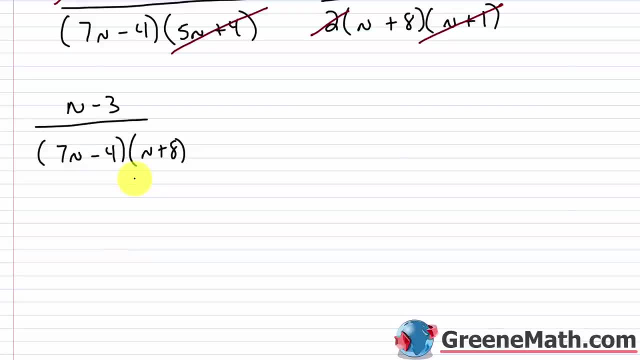 But she might want you to do it. It doesn't matter. It's the same thing either way. So if she asks for it, do it. If not, you can just stop. 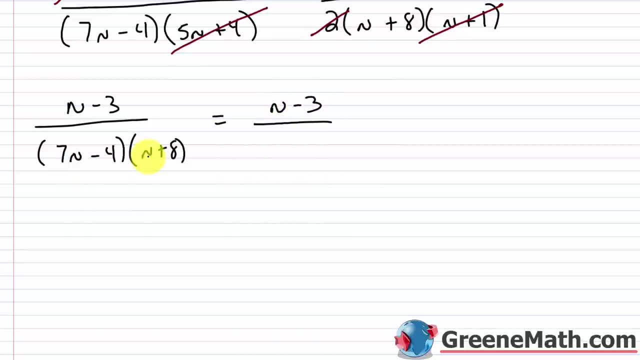 So this is n minus 3 over 7n times n is 7n squared. The outer would be positive 56n. The inner would be negative 4n. So this would be plus 52n. And then the last negative 4 times 8 is negative 32. So you get n minus 3 over 7n squared plus 52n minus 32. 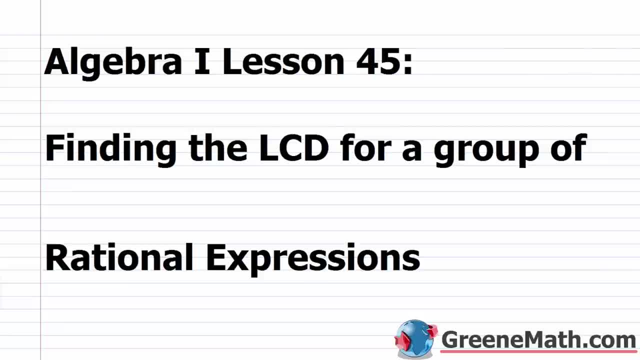 Hello and welcome to Algebra 1 Lesson 45. In this video, we're going to learn about finding the LCD, that's the least common denominator, for a group of rational expressions. 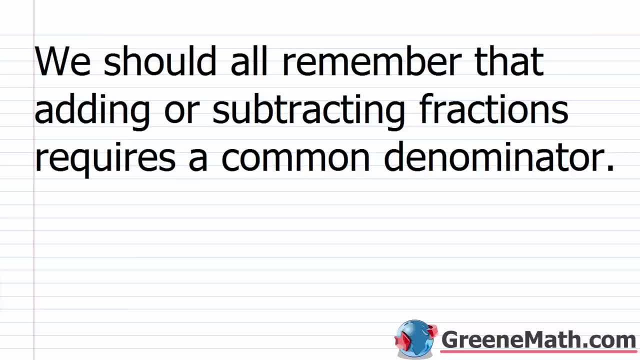 So now that we've mastered how to multiply and divide rational expressions, kind of the next thing we're going to learn is how to add and subtract rational expressions. 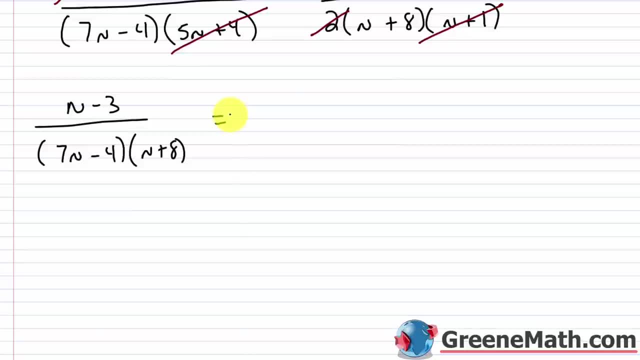 same thing either way. So if she asks for it, do it, If not, you can just stop. So this is n minus 3 over 7n times. n is 7n squared, The outer would be positive 56n. 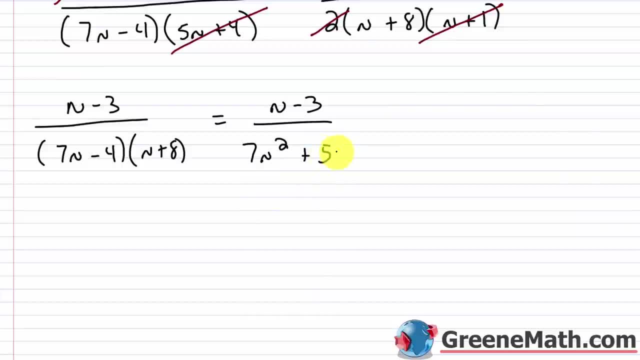 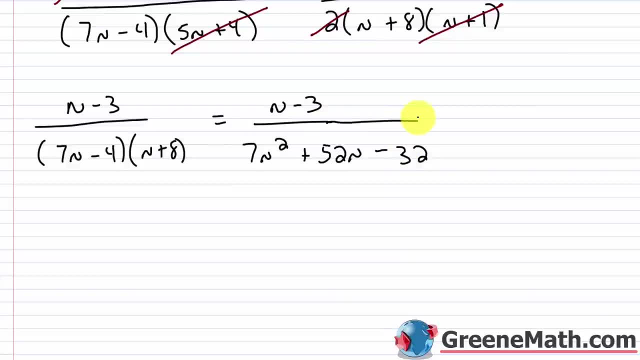 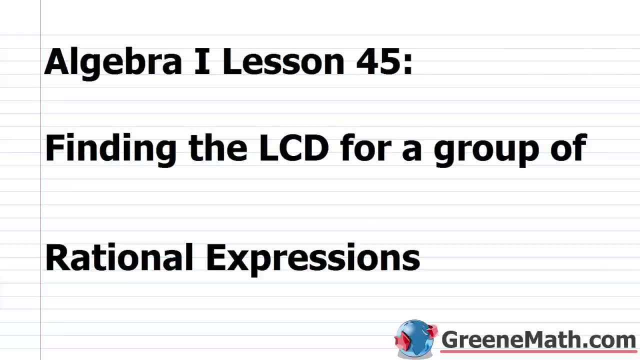 is negative 32.. So you get n minus 3 over 7n squared, plus 52n minus 32.. Hello and welcome to Algebra 1, Lesson 45.. In this video we're going to learn about finding the LCD. that's the least. 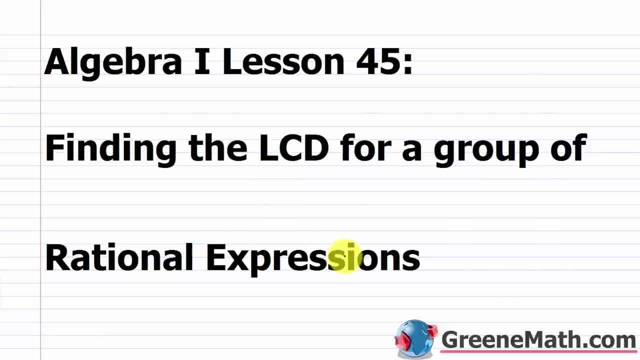 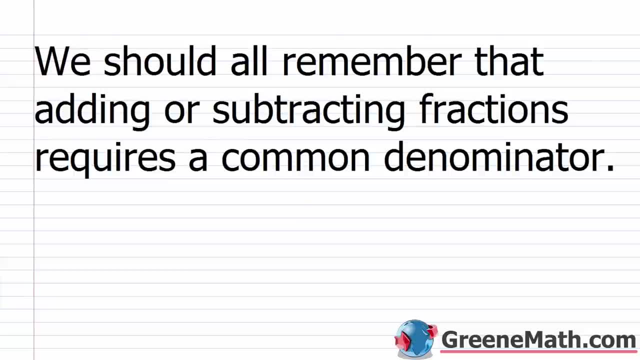 common denominator for a group of rational expressions. So now that we've mastered how to multiply and divide rational expressions, kind of, the next thing we're going to learn is how to add and subtract rational expressions. Now, before we can do that, we need to learn how to find the 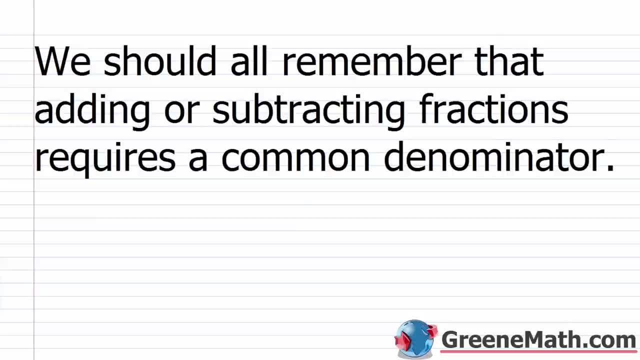 least common denominator for a group of rational expressions. So I want you to think back to when we worked with fractions in pre-algebra And we should all remember that adding or subtracting fractions requires a common denominator, And you want to find the least common denominator. 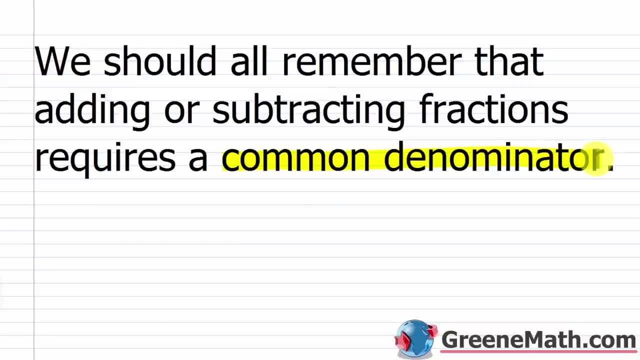 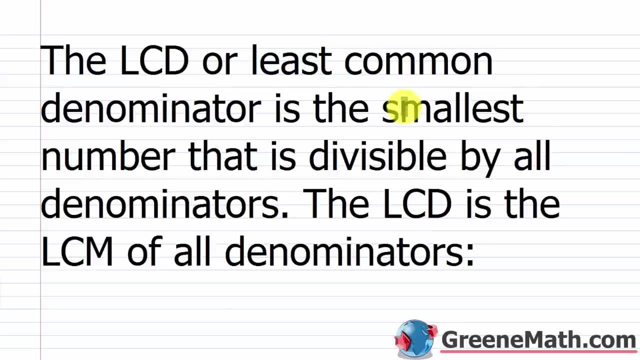 because that's going to save you time and effort with regard to your simplification in the end. So the LCD, or least common denominator, is the smallest number that is divisible by all denominators. The LCD is the LCM of all denominators. Now let me kind of explain this. 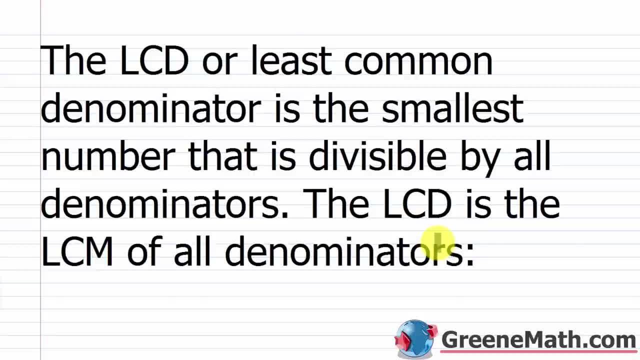 A lot of students get confused when you start talking about LCD and LCM and GCF and GCD. They always get those confused for the first part of kind of their math career. So the LCM is the least common denominator. So you have two, three, four numbers, whatever it is, and you want to find 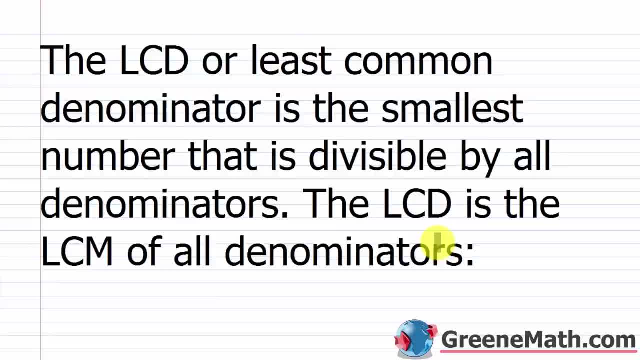 the least common multiple. When we talk about the least common denominator, that's when we're working with fractions And we just take the denominators and we find the least common multiple of the denominators and that is the LCD. So you can see how the LCM and the LCD are. 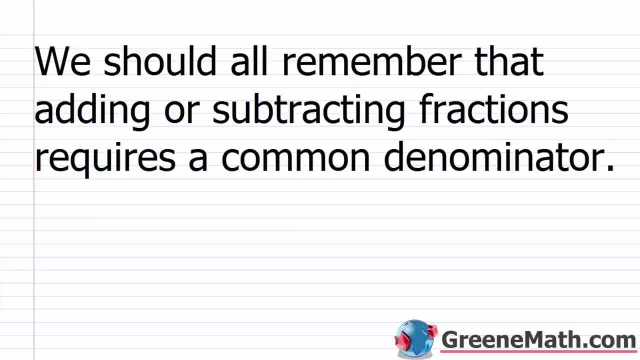 Now, before we can do that, we need to learn how to find the least common denominator for a group of rational expressions. 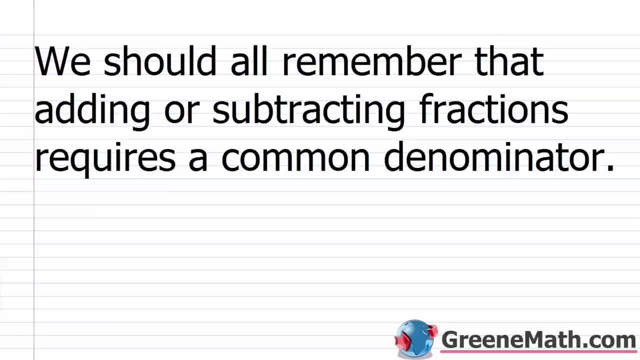 So I want you to think back to when we worked with fractions in pre-algebra. And we should all remember that adding or subtracting fractions requires a common denominator. 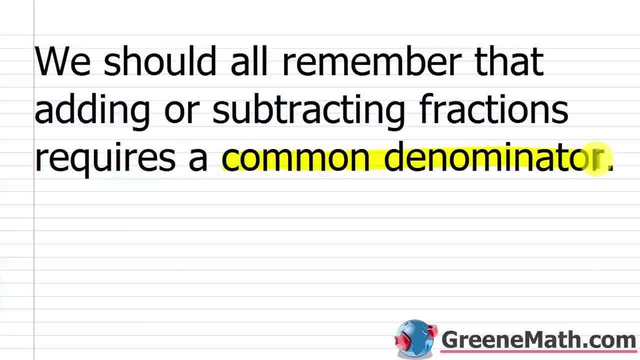 And you want to find the least common denominator because that's going to save you time and effort with regard to your simplification in the end. 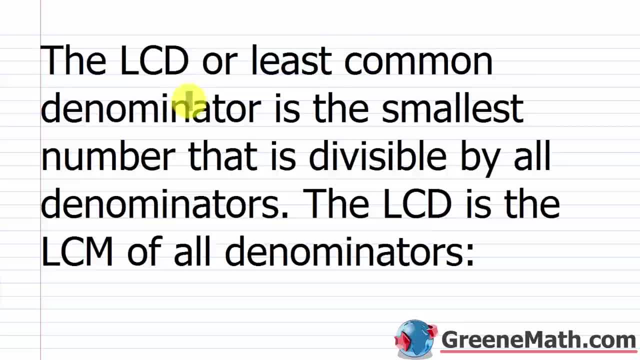 So the LCD, or least common denominator, is the smallest number that is divisible by all denominators. The LCD is the LCM of all denominators. 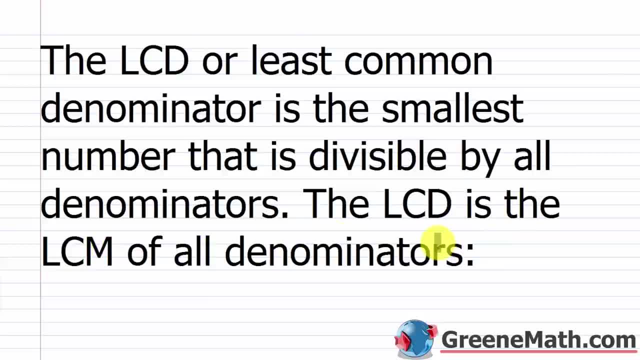 Now, let me kind of explain this. A lot of students get confused when you start talking about LCD and LCM and GCF and GCD. 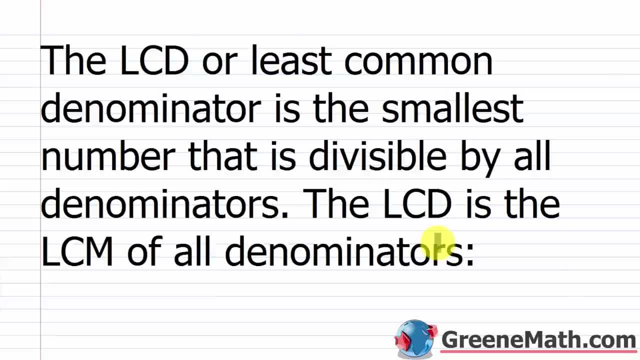 They always get those confused for the first part of kind of their math career. 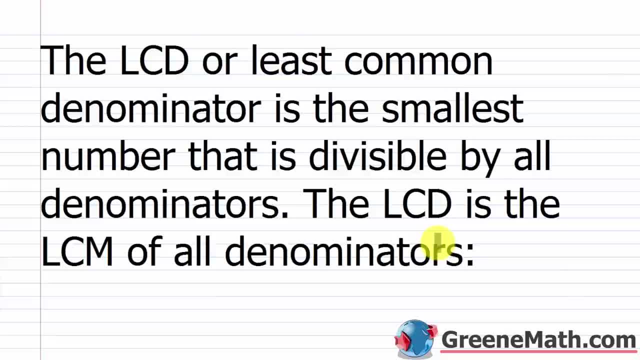 So the LCM is the least common multiple. So you have two, three, four numbers, whatever it is, and you want to find the least common multiple. When we talk about the least common denominator, that's when we're working with fractions, and we just take the denominators and we find the least common multiple of the denominators, and that is the LCD. So you can see how the LCM and the LCD are related. 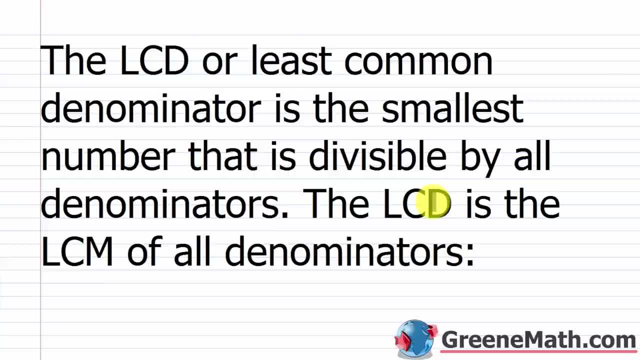 Now, the greatest common factor, or the greatest common divisor, those are the same thing. If something is a factor, it's also a divisor. When we talk about that, we're looking for a number that is the largest factor or the largest divisor of a group of numbers. 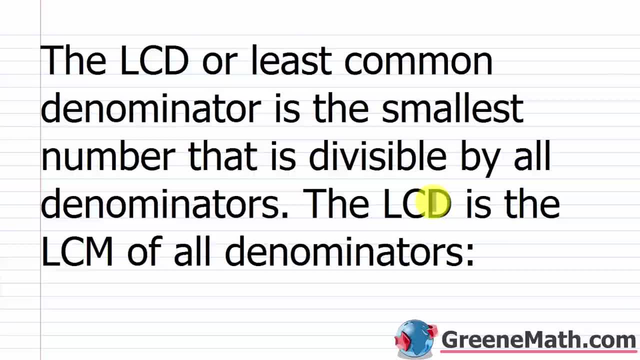 Now, the way they're different is that the GCF or the GCD is going to generally be a smaller number, 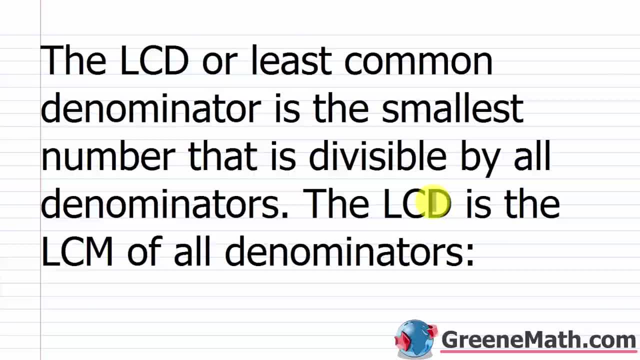 and the LCM or the LCD is going to be a larger number. 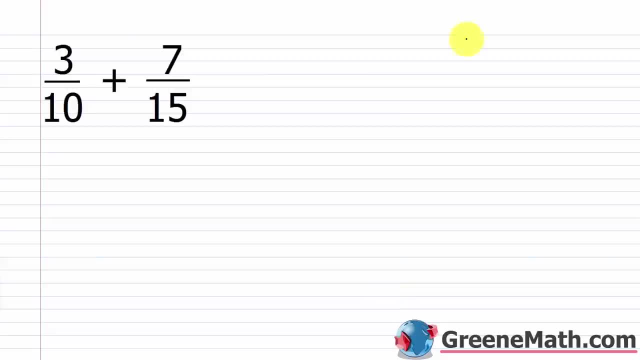 So let's revisit real quick with this example with adding fractions. So I have something like 3 tenths plus 7 fifteenths. 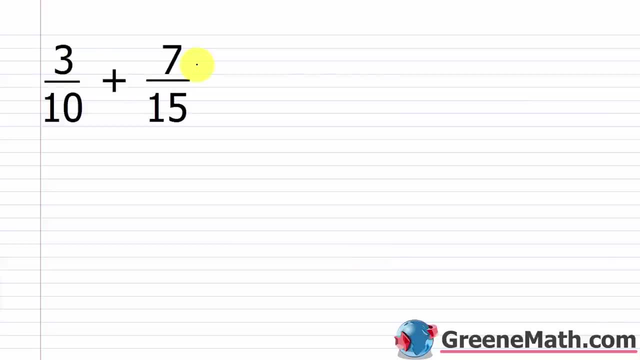 Now, we know that we can't just add across like we do with multiplication, 3 plus 7 is 10, 10 plus 15 is 25. 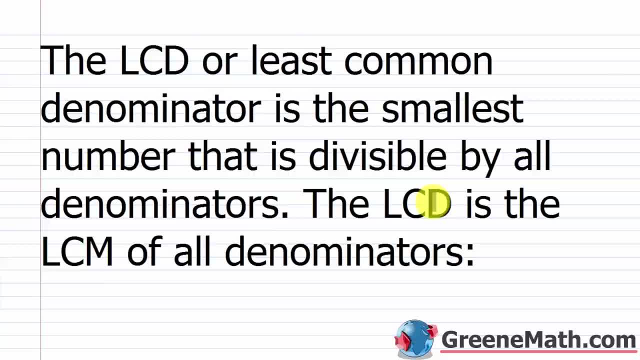 related. Now, the greatest common factor or the greatest common divisor, those are the same thing. Okay, if something is a factor, it's also a divisor. So when we're talking about the least common number, we're looking for a number that is the largest factor or the largest divisor of a group of. 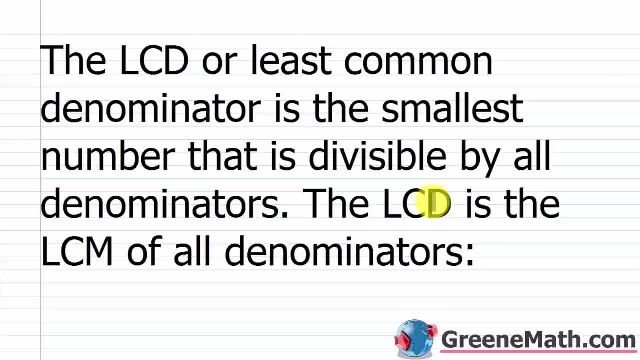 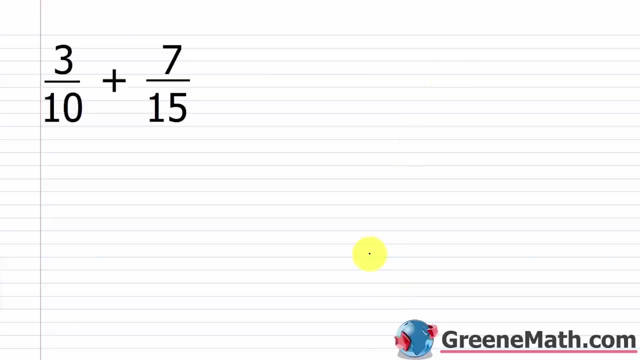 numbers. Now the way they're different is that the GCF or the GCD is going to generally be a smaller number And the LCM or the LCD is going to be a larger number. So let's revisit real quick with this example, with adding fractions, So I have something like three-tenths plus seven-fifteens. 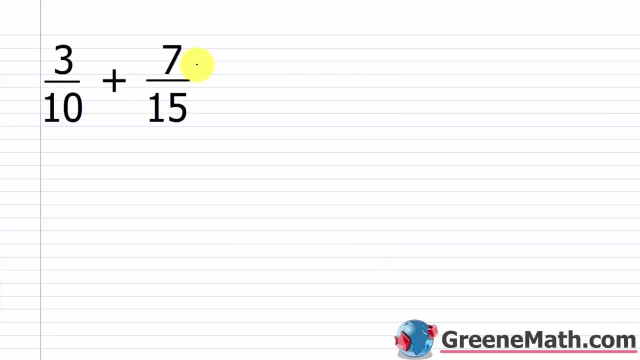 Now we know that we can't just add across like we do with multiplication: three plus seven is 10,, 10 plus 15 is 25.. You know I see students do that. That's wrong. That is wrong. We need to have a common denominator before we start, And the most. 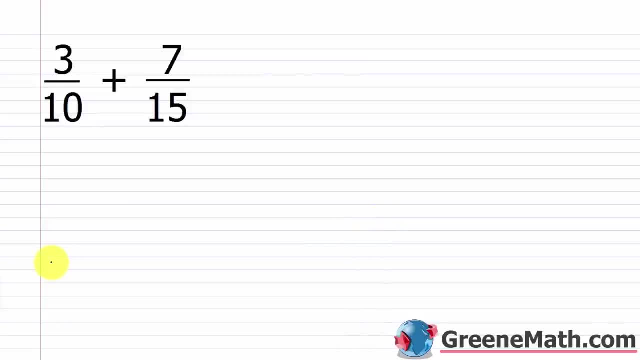 efficient common denominator is the least common denominator, So the LCD, or the least common denominator, And this is equal to the least common multiple of the denominator, So of 10 and 15.. Now hopefully you remember how to do this from pre-algebra, But if you don't, you basically just factor each. 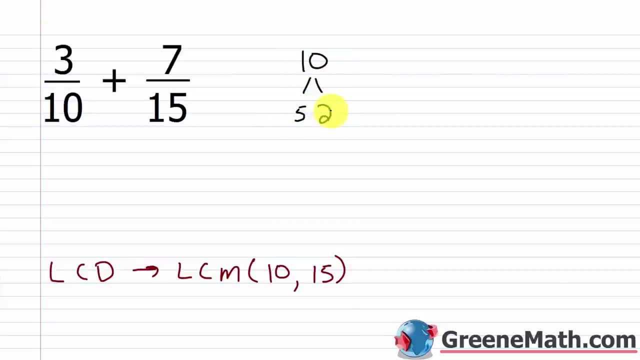 number. So for 10, it's 5 times 2,, 5 is prime, and so is 2.. For 15, it's what it's 5 times 3, 5 is prime, and so is 3.. Now each prime factor from every prime factorization is going to go. 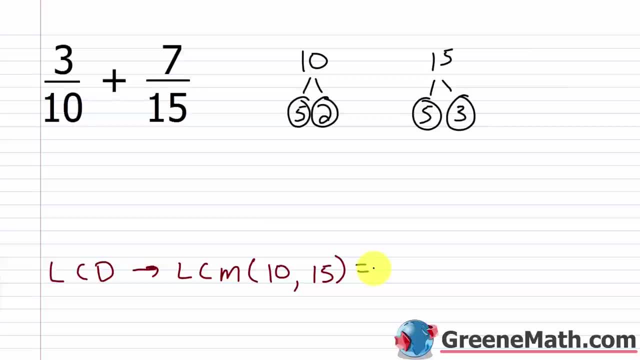 in your list when you build it. The only thing is, if you have a duplicate prime factor, it's only going to go in the largest number of times it occurs either of the factorizations. So in other words, I have five and I have two, I have five and I have. 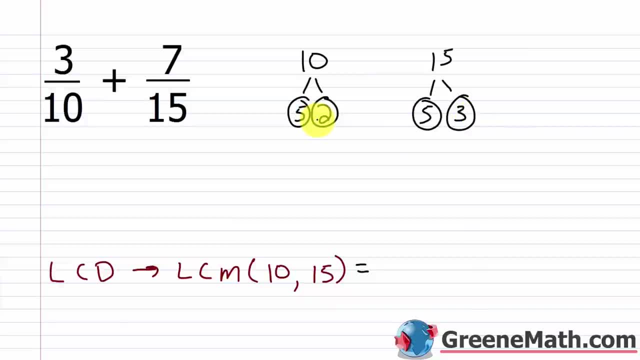 three, So five occurs in each prime factorization. The largest number of repeats or the largest number of occurrences in any of the prime factorizations is one. Just have one here and I have one here, So I'm just going to put one in one factor of five in when I build that. 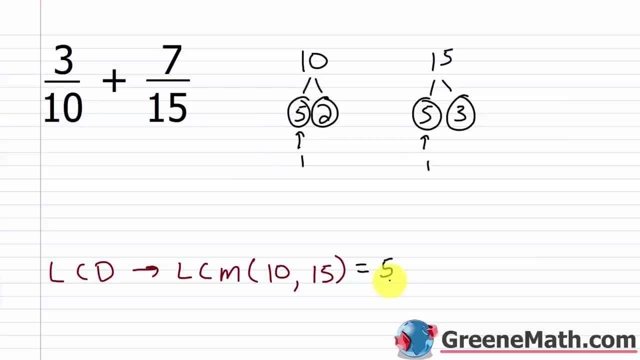 LCM or LCD or however you want to think about it. Now I'm going to multiply by. I have a two here, no two over here, so I just throw it in there. I have a three here, no three over here, so I just. You know, I see students do that. That's wrong. 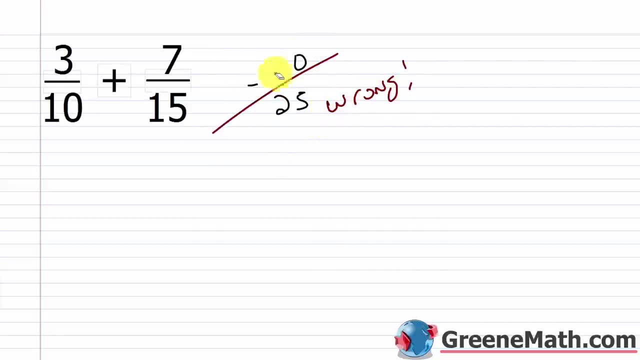 That is wrong. We need to have a common denominator before we start. 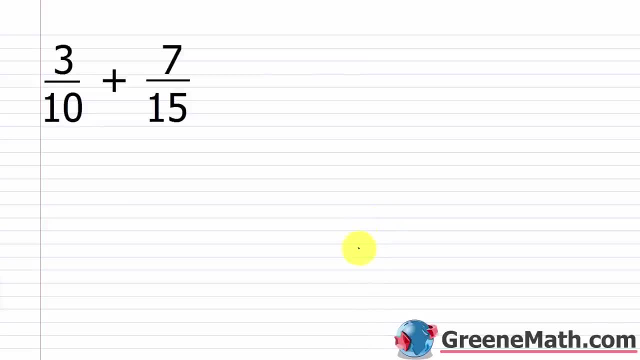 And the most efficient common denominator is the least common denominator, so the LCD, or the least common denominator. And this is equal to 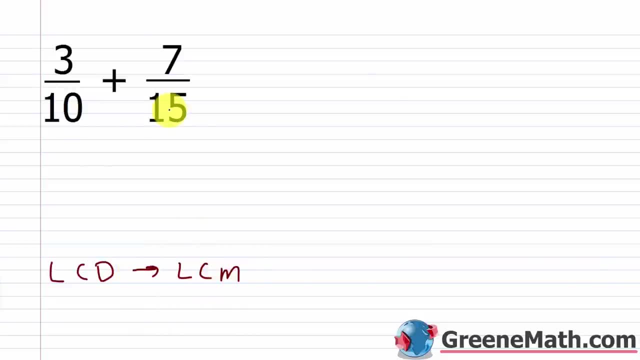 the least common multiple of the denominators, so of 10 and 15. 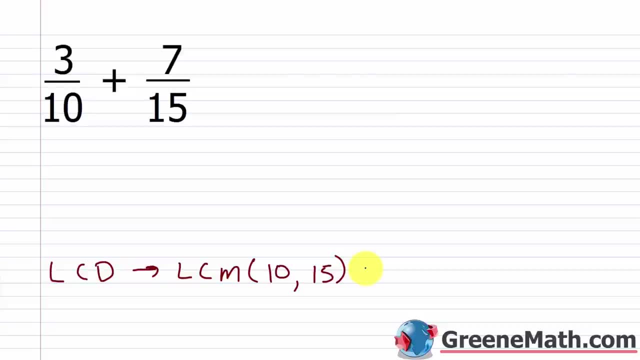 Now, hopefully you remember how to do this from pre-algebra, but if you don't, you basically just factor each number. 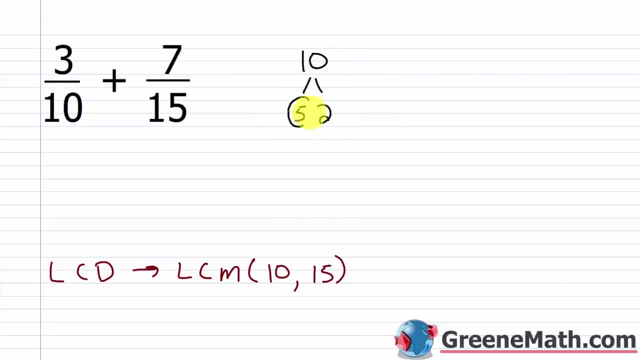 So for 10, it's 5 times 2. 5 is prime and so is 2. For 15, it's what? It's 5 times 3. 5 is prime and so is 3. 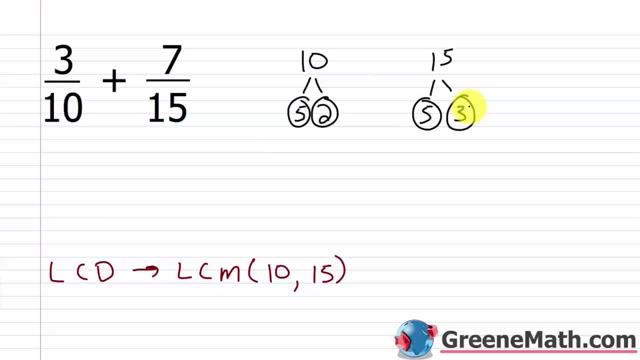 Now, each prime factor from every prime factorization is going to go in your list when you build it. 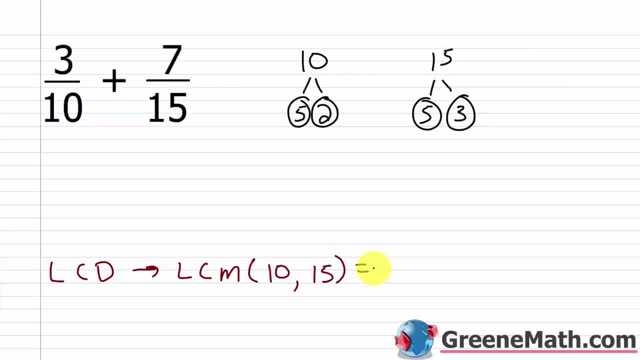 The only thing is, if you have a duplicate prime factor, it's only going to go in the largest number of times it occurs in either of the factorizations. 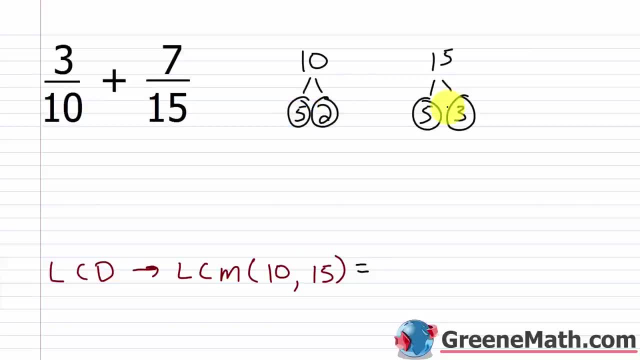 So in other words, I have 5 and I have 2. 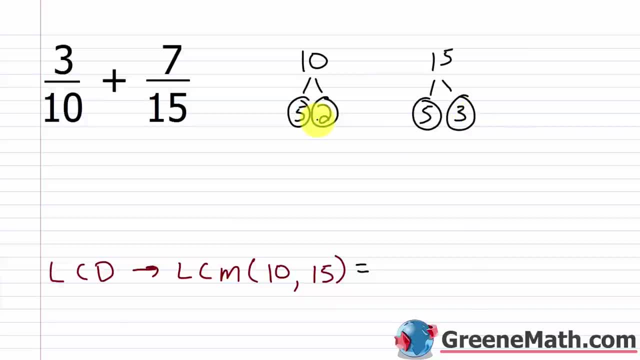 I have 5 and I have 3. So 5 occurs in each prime factorization. The largest number of repeats or the largest number of occurrences 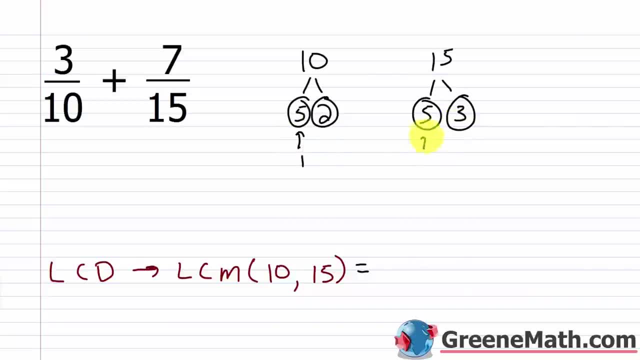 in any of the prime factorizations is 1. I just have 1 here and I have 1 here. 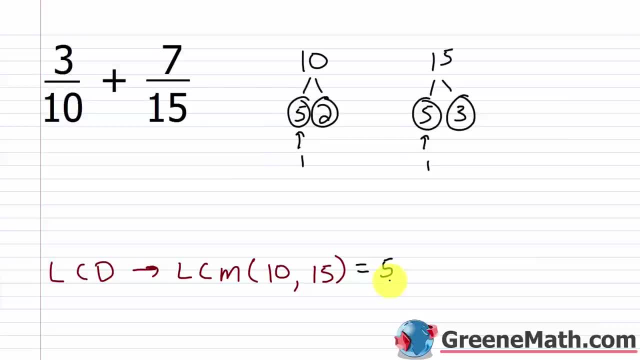 So I'm just going to put 1 in, 1 factor of 5 in, when I build that LCM or LCD or however you want to think about it. 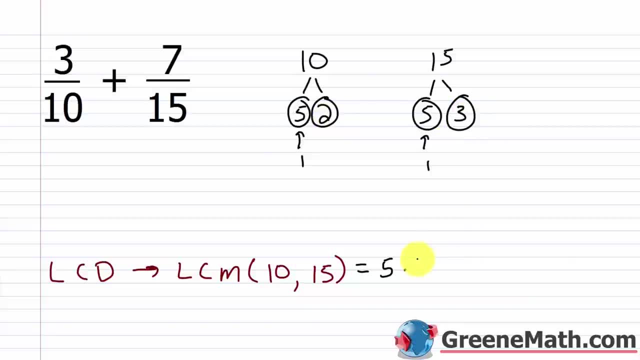 Now, I'm going to multiply by, I have a 2 here, no 2 over here, so I just throw it in there. I have a 3 here, no 3 over here, so I just throw that in there. So the LCD, again, 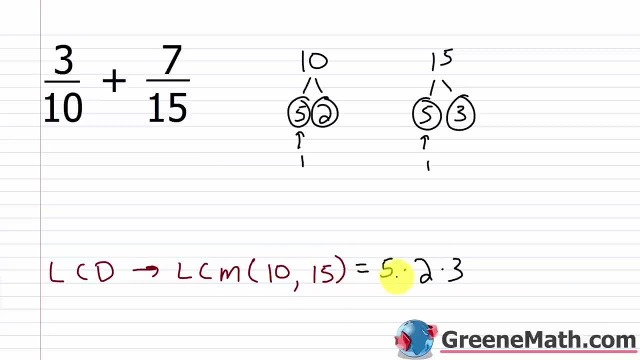 is the LCM, the least common multiple of 10 and 15, and that's 5 times 2, which is 10, times 3, which is 30. 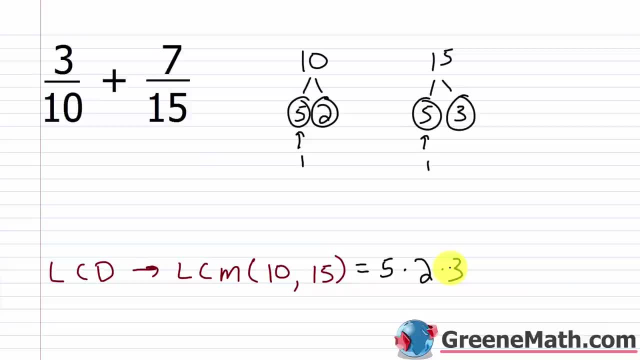 throw that in there. So the LCD again is the LCM, the least common multiple of 10 and 15, and that's five times two, which is 10,, times three, which is 30. So once I have found that, 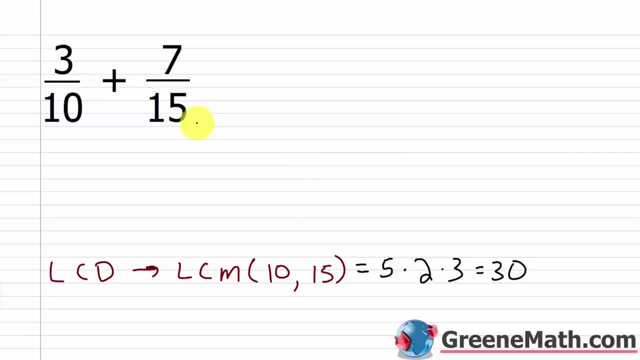 I go through and I rewrite each fraction as an equivalent fraction, where 30 is the denominator. So in other words, with three tenths, I would multiply the numerator by three and also the denominator. Remember, I'm just multiplying by a complicated form of one. 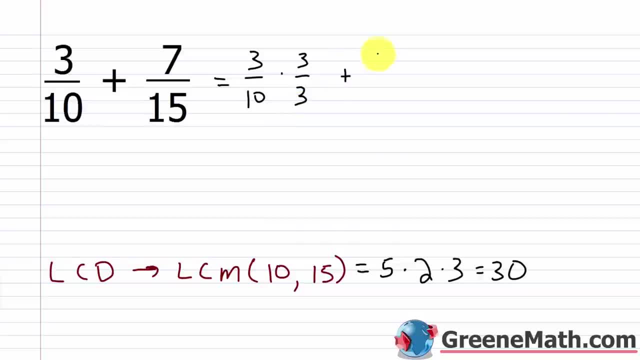 so I'm not changing the value, I'm just changing what it looks like. Then, plus, we have seven, fifteenths, and this is multiplied by two over two, And so this is equal to three times three, is nine over 10 times three, that's 30. Then plus seven times two is 14,. 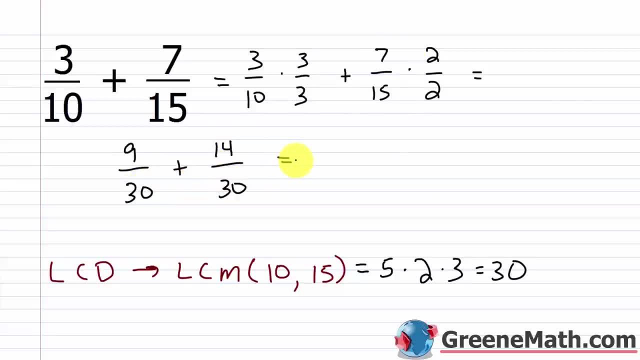 over 15 times two, that's 30. And then nine plus 14 is going to be 23.. So we end up with 23 over 30, as my answer, and that can't be simplified any further. Okay, So we know how to find the LCD with regard to regular fractions. 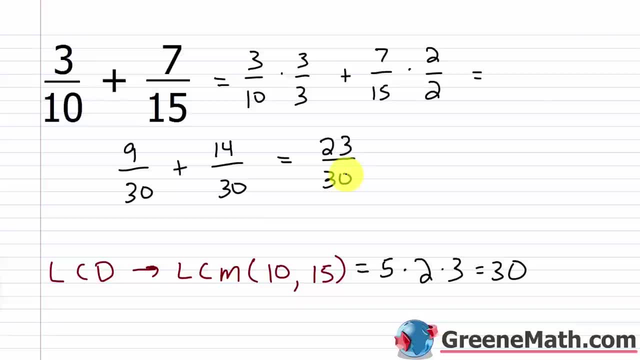 It's going to get a little bit more complicated when we start thinking about rational expressions, because we have some messy variables involved, Right, so it's a little bit more complex, but the general idea is the same. Now, before I move on, 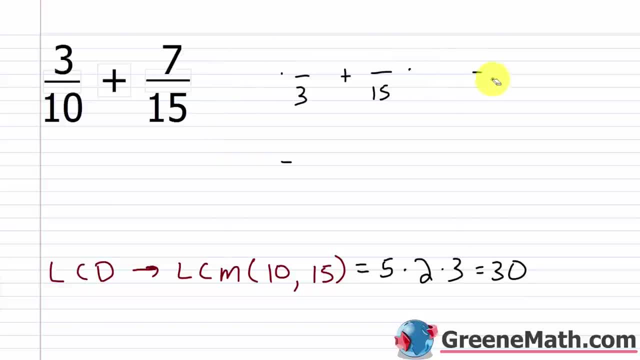 I just want to show you, so that I settle all confusion, that this is not the same as the GCF. Now notice how you have the number 10, and you have the number 15.. Now the LCD, or the LCM, is a larger number. 30 is the smallest positive. 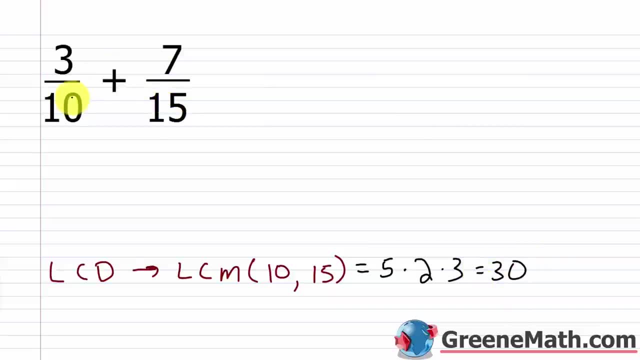 number that is divisible by both 15 and 10, meaning I divide 30 by 15, I get two- no remainder. I divide 30 by 10, I get three- no remainder. okay, If we talk about the greatest common factor. 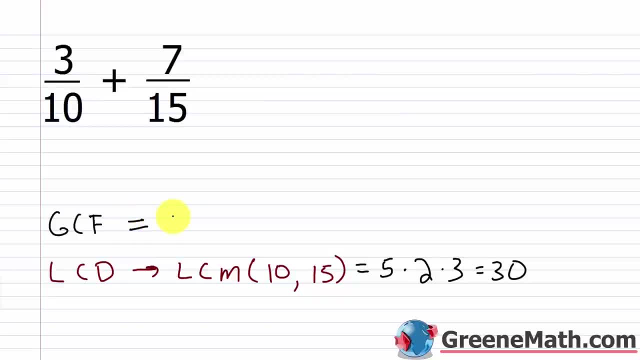 or the greatest common divisor. this is equal to what It's going to be- a smaller number, because we're looking for the largest number that each of these numbers is divisible by. So it's kind of the same process. You factor each number to start, but all you're going to do is look for what's 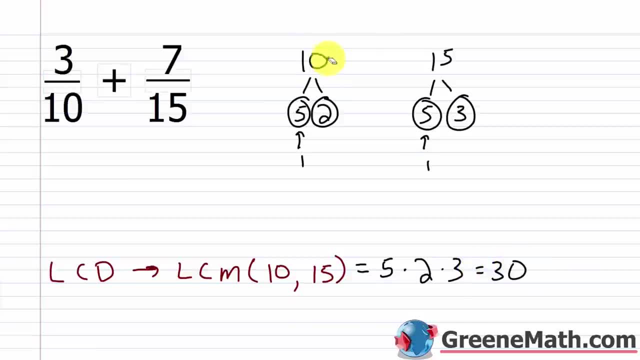 So once I have found that, I go through and I rewrite each fraction as an equivalent fraction where 30 is the denominator. So in other words, with 3 tenths, I would multiply the numerator by 3 and also the denominator. Remember, I'm just multiplying by a complicated form of 1, so I'm not changing the value, I'm just changing what it looks like. 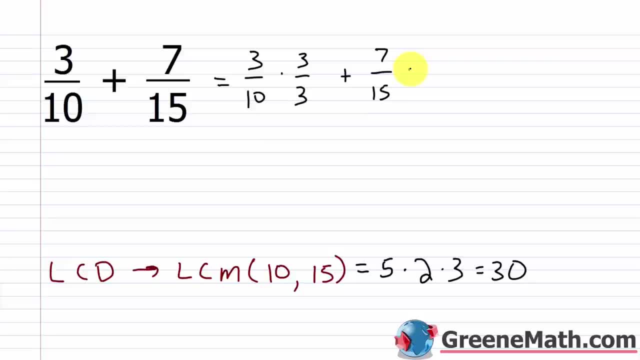 Then plus, we have 7 fifteenths, and this is multiplied by 2 over 2. And so this is equal to 3 times 3 is 9, over 10 times 3, that's 30. Then plus, 7 times 2 is 14, over 15 times 2, that's 30. And then 9 plus 14 is going to be 23. So we end up with 23 over 30 as my answer, and that can't be simplified any further. 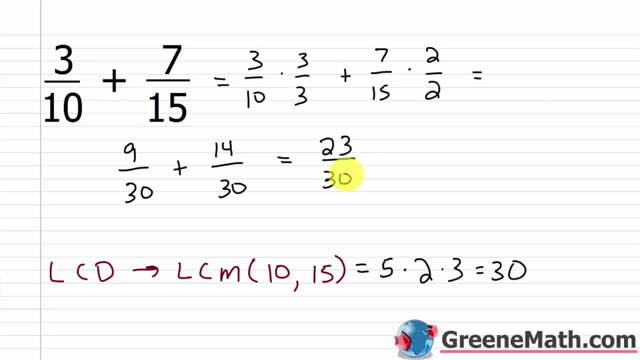 Okay, so we know how to find the LCD with regard to regular fractions. It's going to get a little bit more complicated when we start thinking about rational expressions because we have some messy variables involved, right? 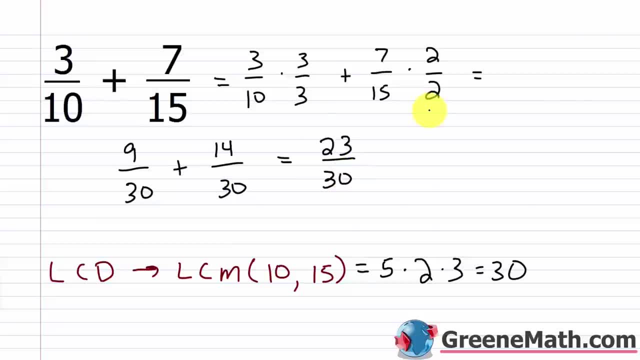 So it's a little bit more complex, but the general idea is the same. 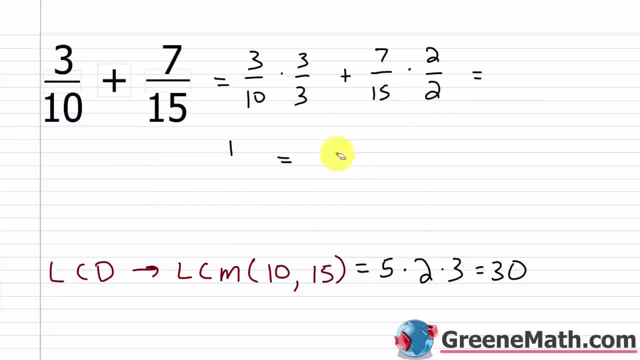 Now before I move on, I just want to show you so that I settle all confusion that this is not the same as the GCF. 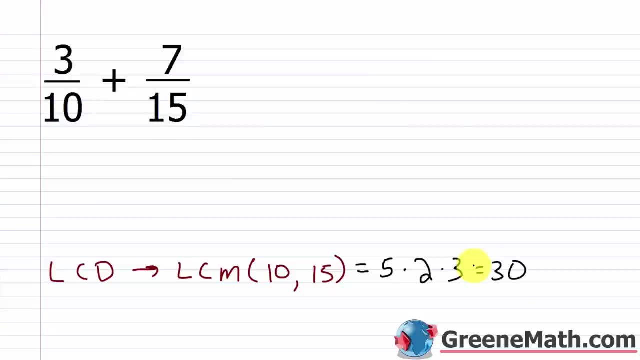 Now notice how you have the number 10 and you have the number 15. Now the LCD or the LCM is a larger number. 30 is the smallest positive number that is divisible by both 15 and 10, meaning I divide 30 by 15, I get 2, no remainder. I divide 30 by 10, I get 3, no remainder. If we talk about the greatest common factor or the greatest common divisor, this is equal to what? It's going to be a smaller number because we're looking for the largest number that each of these numbers is divisible by. 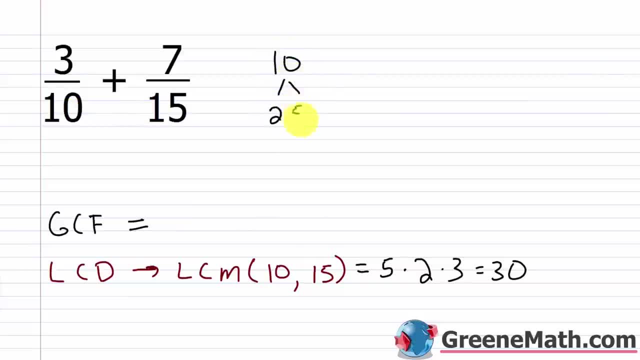 So it's kind of the same process. You factor each number to start, but all you're going to do is look for what's common to both, okay? So I can only put something in the greatest common factor listing if it's common to everything. In this case, I don't have a 2 that's common to everything. I don't have a 3 that's common to everything. 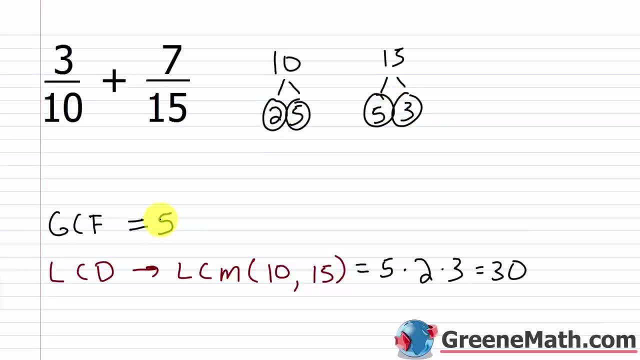 The only thing that's common to both is 5, and so my greatest common factor is a 5. 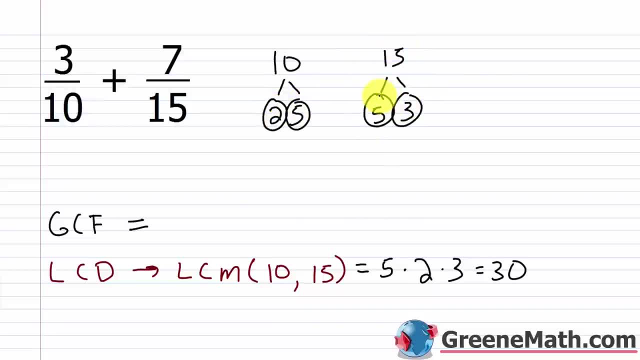 common to both. okay, So I can only put something in the greatest common factor listing if it's common to everything. In this case, I don't have a two that's common to everything. I don't have a three that's common to everything. The only thing that's common to both is five, And so my greatest. 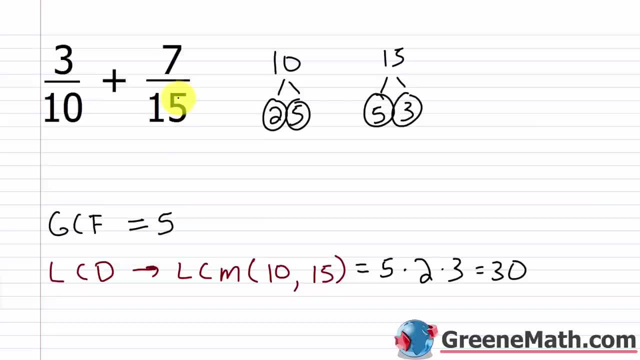 common factor is a five. 10 divided by five is two, no remainder. I divide 30 by 10, I get three, no remainder. 15 divided by five is three- no remainder. So you see that the greatest common factor, or again the greatest common divisor, is a smaller number And the LCD or LCM is a larger 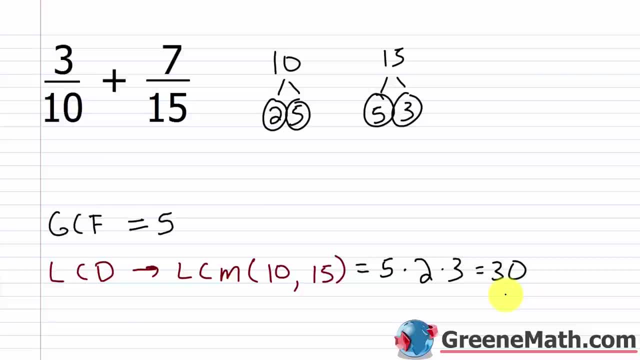 number. So that's one of the tricks I used to remember. It was taught to me by a teacher back when I was in eighth grade, But it's something that you should think about because a lot of students really struggle with this definition between, again, the GCF and the GCD- same thing. 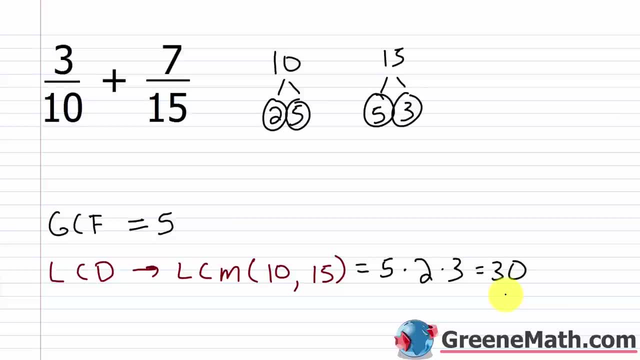 and then the LCD, the least common denominator, which is the LCM of the denominators. So let's look at one more example with fractions, real quick, just to kind of get our feet going. We have 11, 24th minus 9, 20th. So again, if I want the LCD, this is the least common multiple. 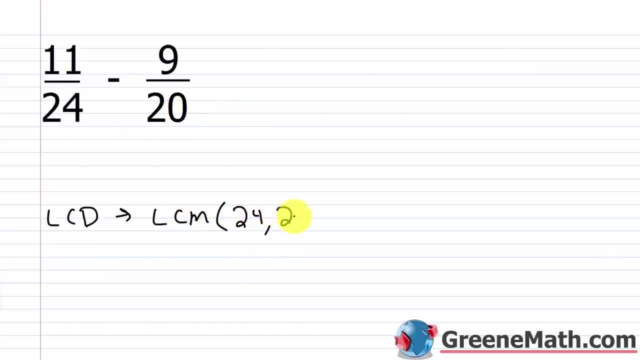 of these two denominators, So of 24 and 20.. So what do I do? I factor 24.. And I could do four times six. four is two times two, six is two times three For 20,. I'll do five times four. 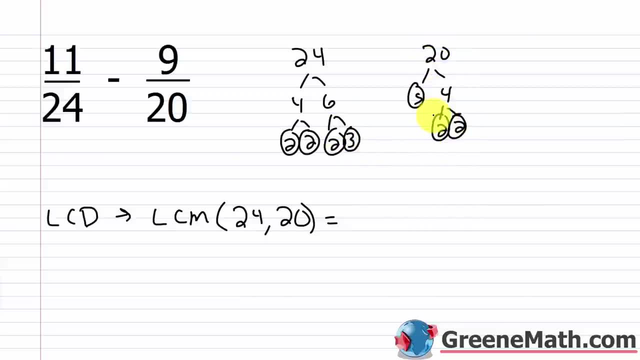 four is two times two. So now if I build my list, every prime factor from each prime factorization is going to go in there. I'm just paying attention for duplicate prime factors. So with two, I have one, two, three of those here And I have one, two of those here. So when I build my list, 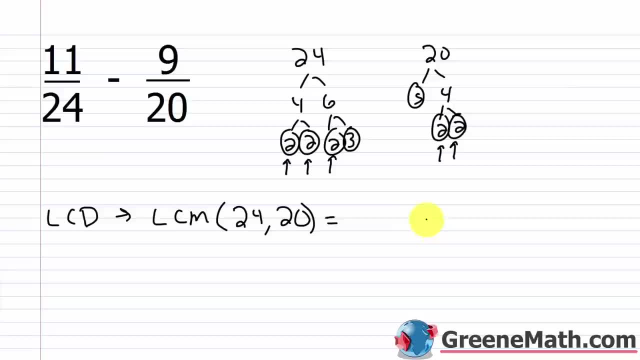 how many am I going to put in here? Well, I'm going to put three. I go with the largest number of repeats from either prime factorization That occurs. here I have two, three, four, five, six, three of them. So I'm going to put two times two times two, or eight Again, where students make a 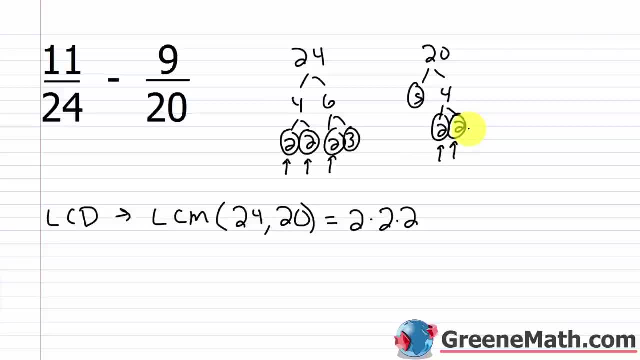 mistake is they throw all of them in there And that's going to give you a common multiple, but it's not going to be the least common multiple. And that's what you're looking for: to reduce the amount of work when you go to simplify. All right, So now the next thing is: I have a three. 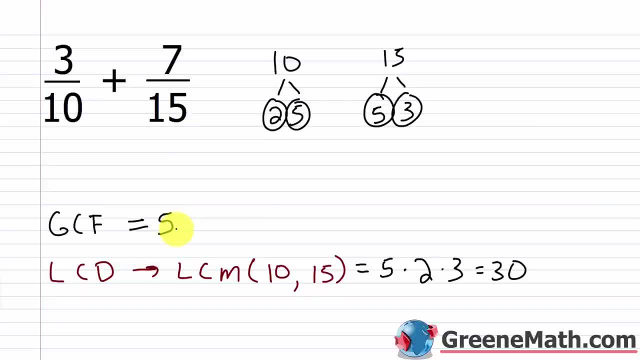 10 divided by 5 is 2, no remainder. 15 divided by 5 is 3, no remainder. 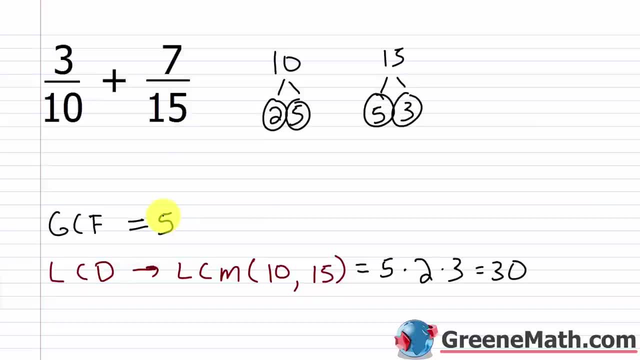 So you see that the greatest common factor, or again, the greatest common divisor, is a smaller number, and the LCD or LCM is a larger number. So that's one of the tricks I used to remember. It was taught to me by a teacher back when I was in eighth grade. 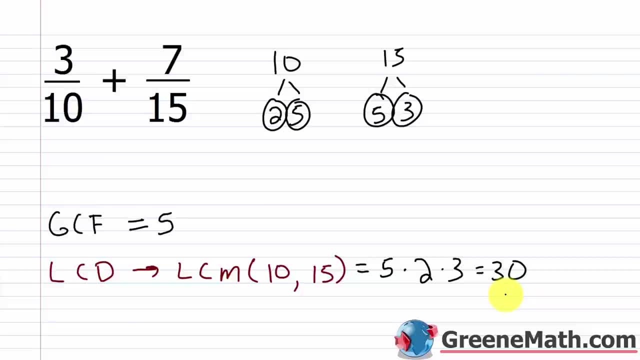 But it's something that you should think about because a lot of students really struggle with this definition between, again, the GCF and the GCD, same thing, and then the LCD, the least common factor, the least common denominator, which is the LCM of the denominators. 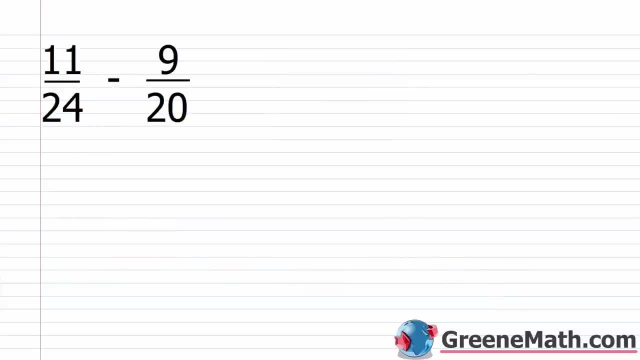 So let's look at one more example with fractions real quick, just to kind of get our feet going. We have 11 24ths minus 9 20ths. 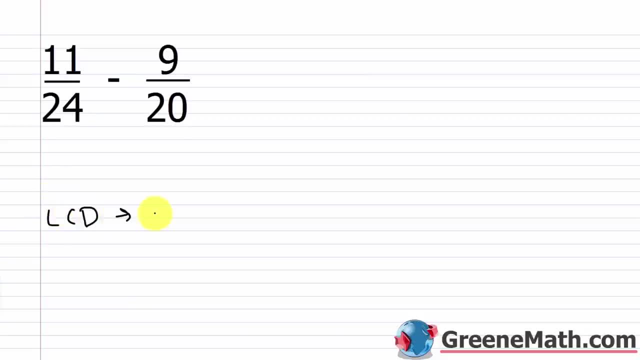 So again, if I want the LCD, this is the least common multiple of these two denominators, 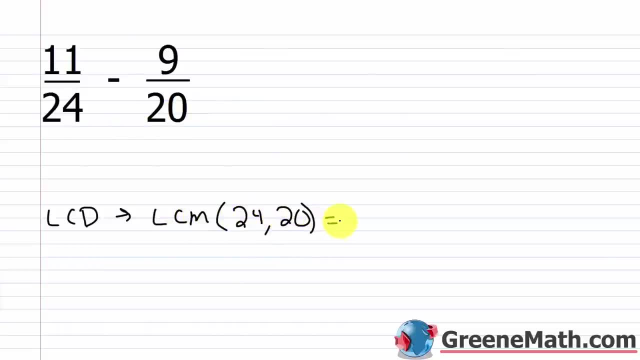 so of 24 and 20. So what do I do? I factor 24, and I can do 4 times 6. 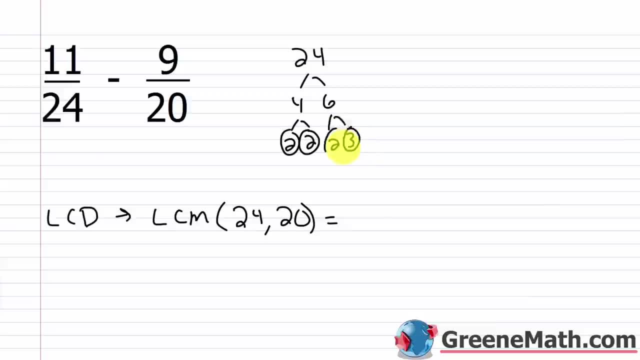 4 is 2 times 2. 6 is 2 times 3. 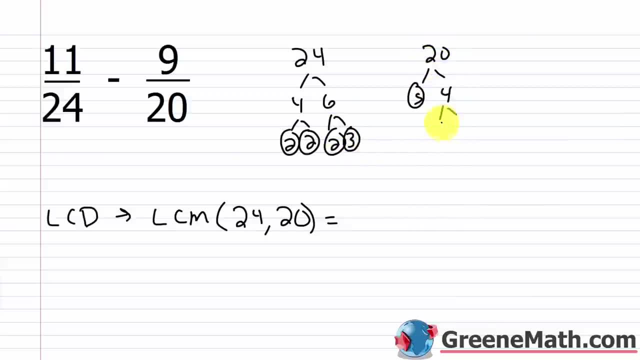 For 20, I'll do 5 times 4. 4 is 2 times 2. 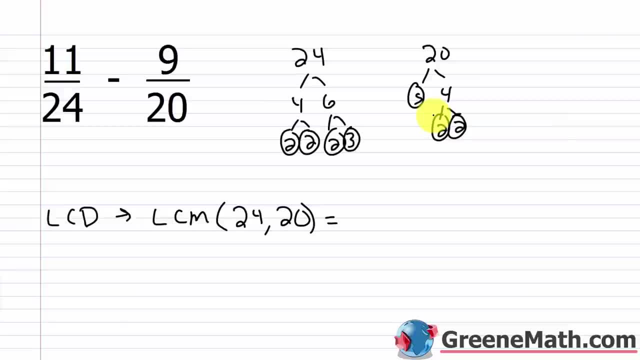 So now, if I build my list, every prime factor from each prime factorization is going to go in there. I'm just paying attention for duplicate prime factors. So with 2, I have 1, 2, 3 of those here, and I have 1, 2 of those here. So when I build my list, how many am I going to put in here? 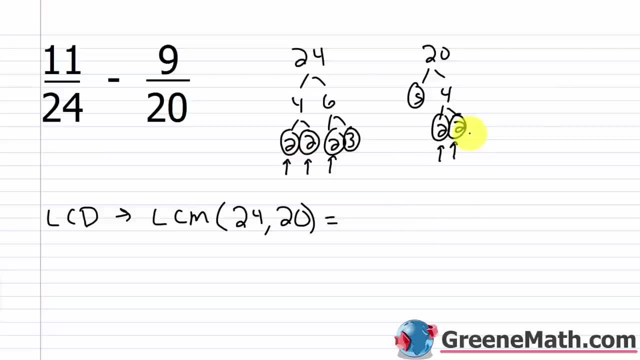 Well, I'm going to put 3. I go with the largest number of repeats from either prime factorization. 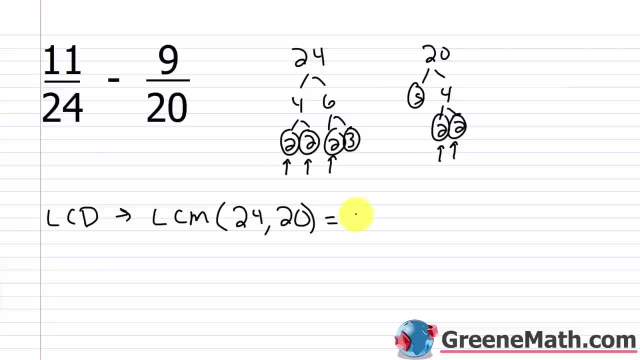 That occurs here. I have 3 of them, so I'm going to put 2 times 2 times 2, or 8. 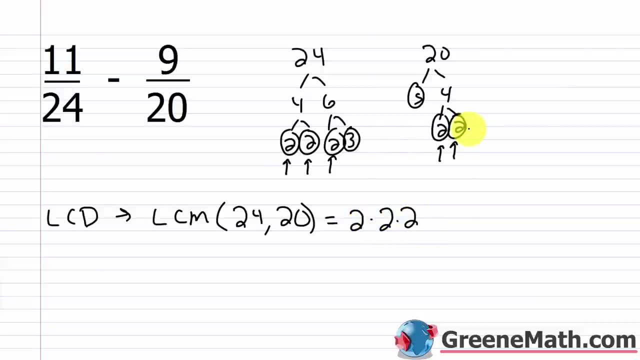 Again, where students make a mistake is they throw all of them in there. And that's going to give you a common multiple, but it's not going to be the least common multiple. And that's what you're looking for to reduce the amount of work 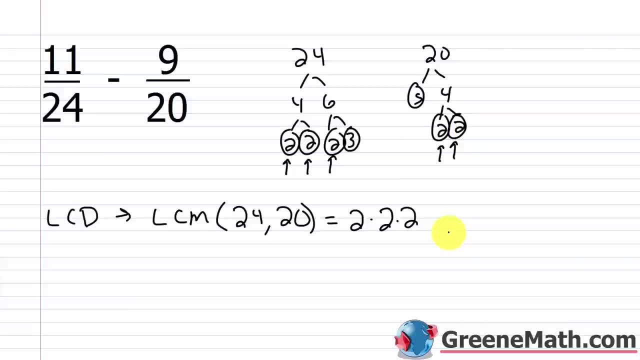 when you go to simplify. Alright, so now, the next thing is I have a 3, not common to both, so I'm going to throw that in there. 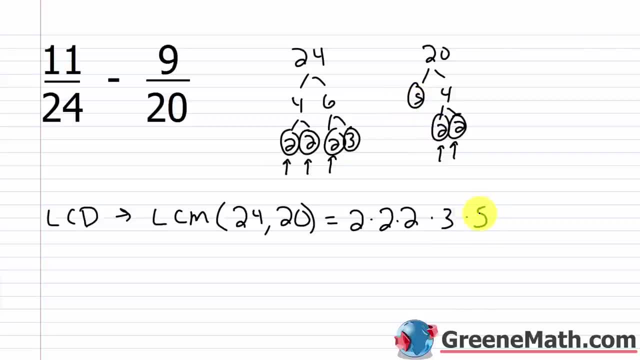 And then I have a 5, not common to both, so I'm just going to throw that in there. 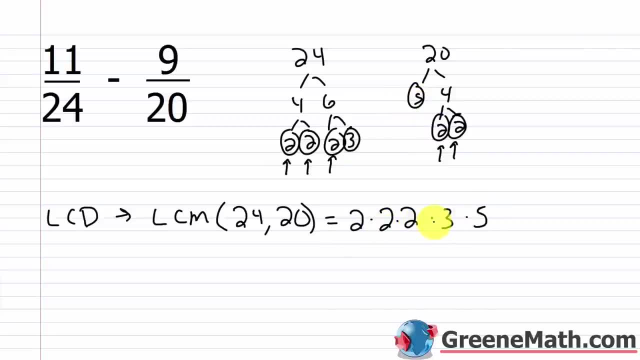 So now we just multiply. 2 times 2 times 2 is 8. 8 times 3 is 24. 24 times 5 is 120. 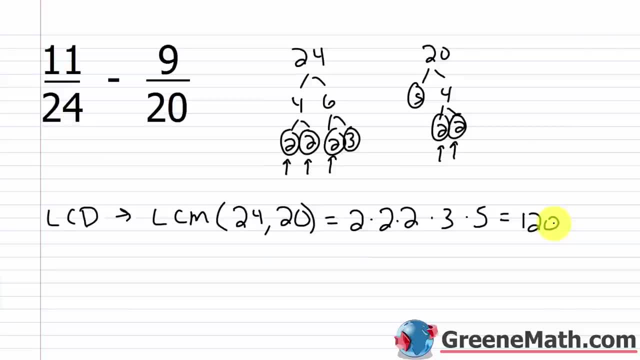 So that's your LCD or LCM. Now, if we wanted to find the GCF, 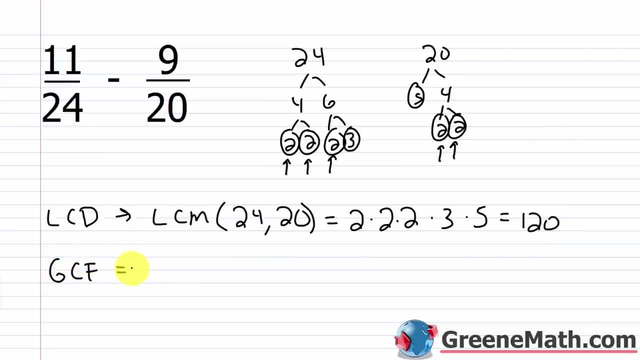 the greatest common factor, or the greatest common divisor, what would that be? Well, when we build that list, it's only going to be numbers in the prime factorizations that's common to everything. The only thing we have here that's common to everything is 2. 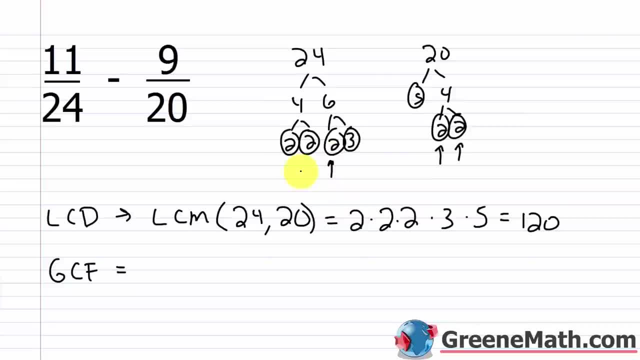 Now, I have 2 factors of 2 here. And again, I have 1, 2, 3 factors of 2 here. With the GCF, it's got to be common to everything. So it's going to be 2 factors of 2 that's going to go into the GCF. And so 2 factors of 2 is 4. So the greatest common factor is 4. 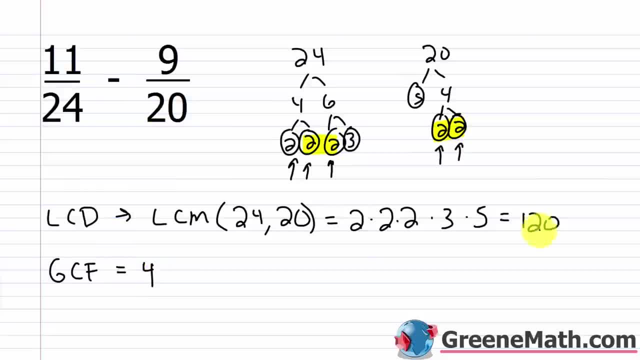 Again, this is a smaller number than these two. And then the LCD or LCM is a larger number than these two. That's how you kind of get an understanding of it. 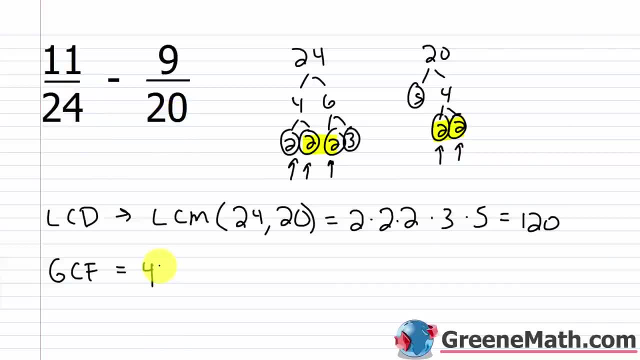 24 divided by 4 is 6. No remainder. 20 divided by 4 is 5. No remainder. With this one, 120 divided by 24 is 5. No remainder. And 120 divided by 20 is 6. No remainder. 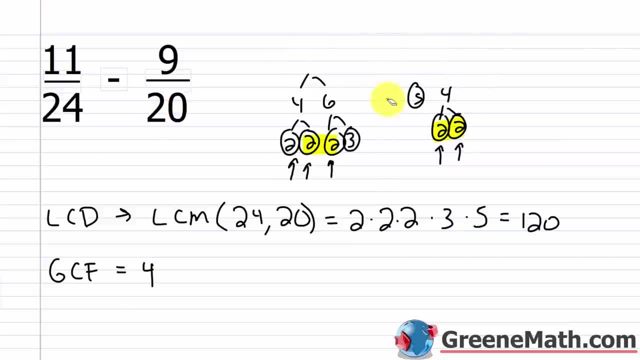 So you can see the difference between the two. Now, let's go ahead and execute this problem just for the sake of completeness. 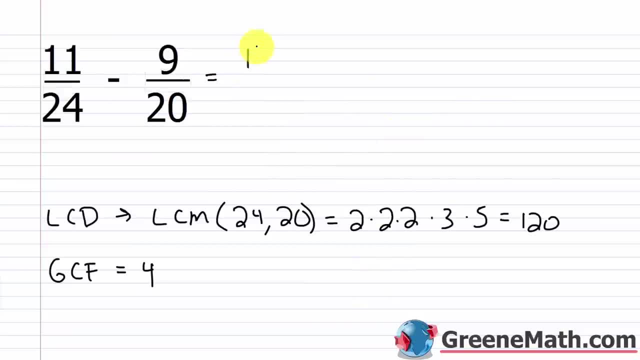 We know what the LCD is, so let's transform each fraction. 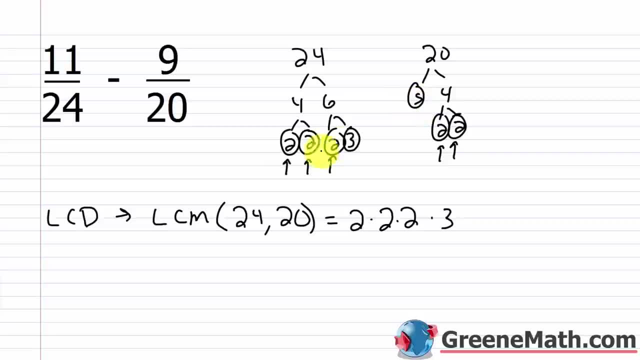 not common to both, So I'm going to throw that in there. And then I have a five not common to both, So I'm just going to throw that in there. So now we just multiply two times. two times two is eight. 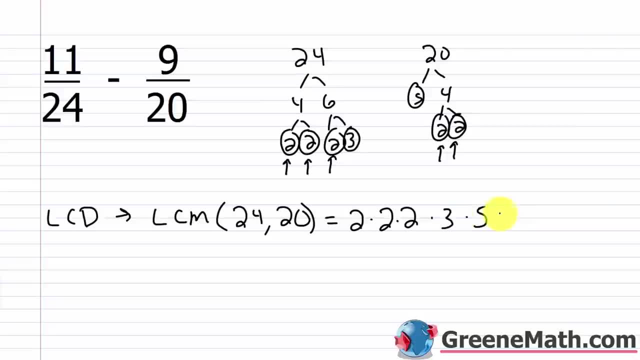 Eight times three is 24.. 24 times five is 120.. So that's your LCD or LCM. Now if we wanted to find the GCF, the greatest common factor or the greatest common divisor, what would that be? But when we build, 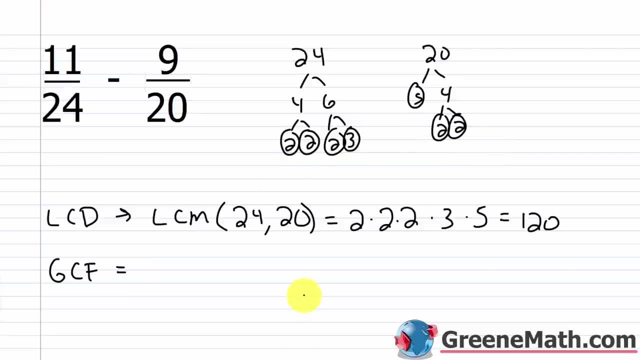 that list. it's only going to be numbers in the prime factorizations. that's common to everything. The only thing we have here that's common to everything is two. Now I have two factors of two here, And again I have one, two, three factors of two here, And I'm going to put two. 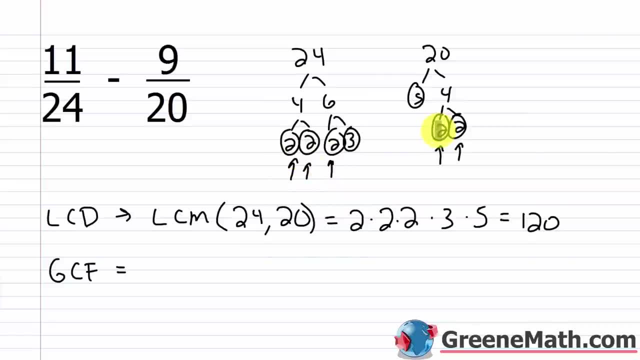 factors of two here. With the GCF it's got to be common to everything, So it's going to be two factors of two That's going to go into the GCF, And so two factors of two is four, So the greatest. 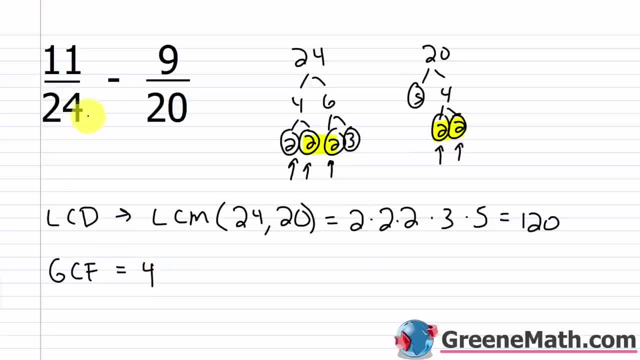 common factor is four. Again, this is a smaller number than these two. And then the LCD, or LCM, is a larger number than these two. That's how you kind of get an understanding of it. 24 divided by four is six- no remainder. 20 divided by four is five, no remainder. With this one, 120 divided. 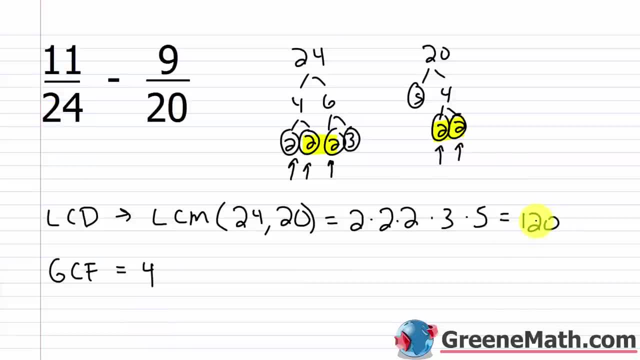 by 24 is five, no remainder. With this one, 120 divided by 24 is five, no remainder. With this one, 120 divided by 24 is six, no remainder. And 120 divided by 20 is six, no remainder. So you can. 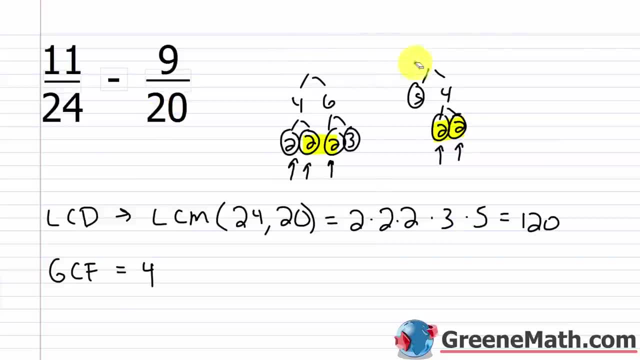 see the difference between the two. Now let's go ahead and execute this problem, just for the sake of completeness. We know what the LCD is, So let's transform each fraction So we'd have 11 over 24.. We'd multiply this by five over five, And then minus nine over 20.. And we'd multiply. 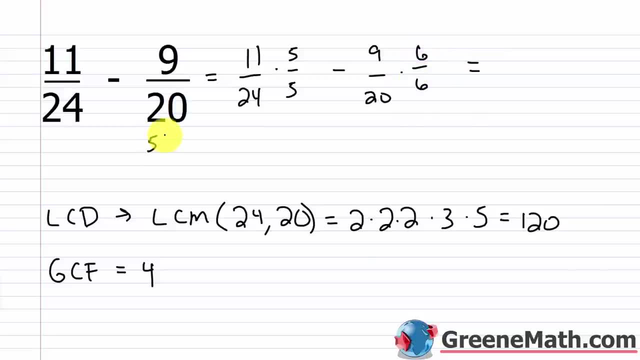 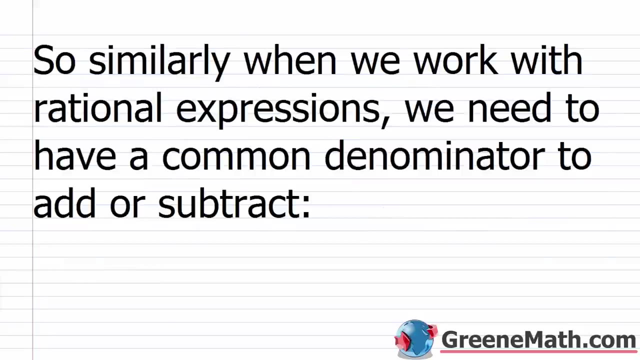 this by six over six, So I'd end up with 55 over 120.. Minus 54 over 120. And this would give me one over 120 as my answer, And I can't simplify that any further. So again, similarly, when we work with rational expressions, we need to have a. 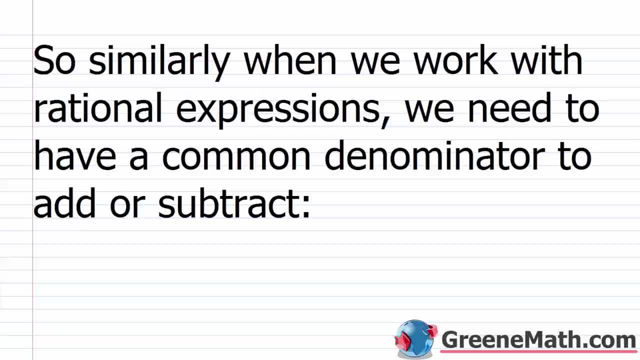 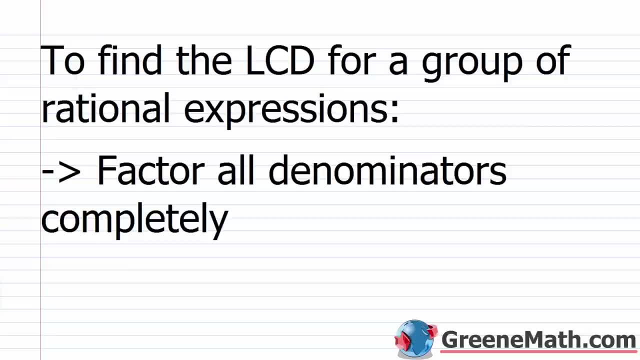 common denominator to add or subtract. It's going to be the same process. Again, it's going to be messier because we have a lot of variables involved. So to find the LCD for a group of rational expressions, we're going to factor all denominators completely, Just like if I'm looking 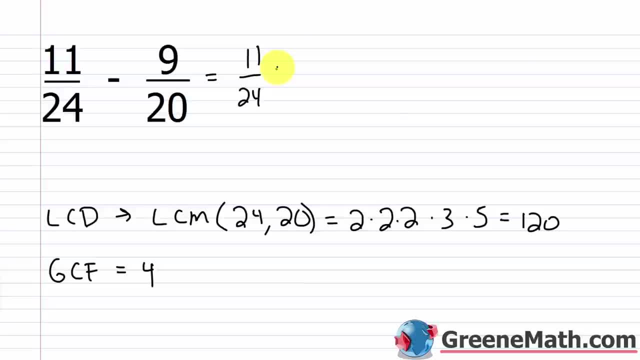 So we'd have 11 over 24. We'd multiply this by 5 over 5 and then minus 9 over 20 and we'd multiply this by 6 over 6. So I'd end up with 55 over 120 minus 54 over 120. And this would give me 1 over 120 as my answer. And I can't simplify that any further. 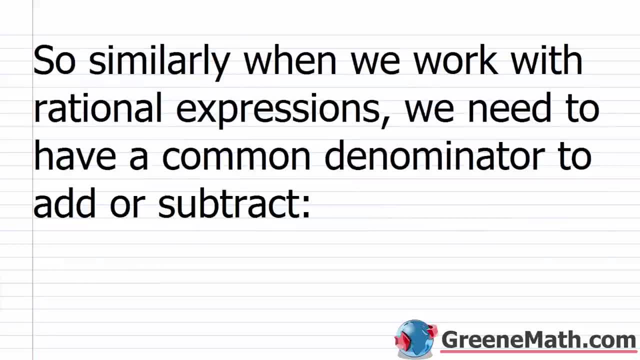 So again, similarly, when we work with rational expressions, we need to have a common denominator to add or subtract. 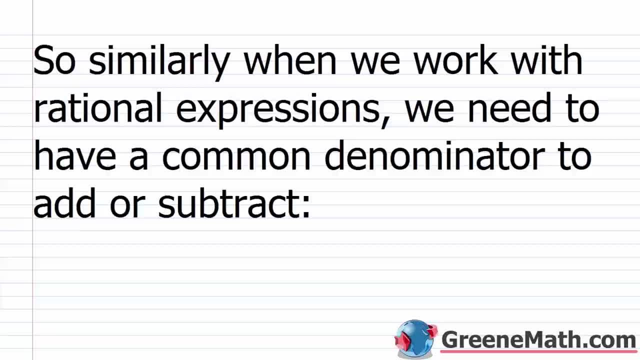 It's going to be the same process. Again, it's going to be messier because we have a lot of variables involved. 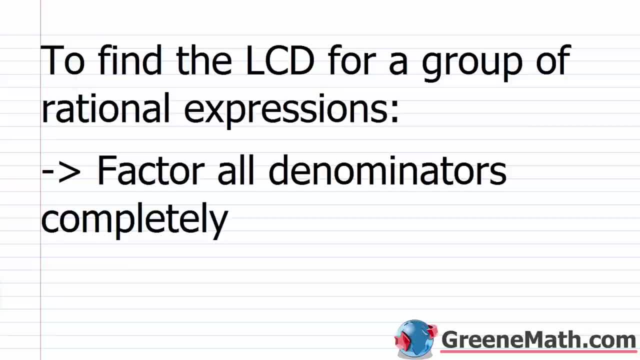 So to find the LCD for a group of rational expressions, we're going to factor all denominators completely. Just like if I'm looking for the LCD for a group of numbers, I'm going to factor the denominators completely. I'm getting it down to the prime factorization of each number. Then I'm going to list each different denominator factor. 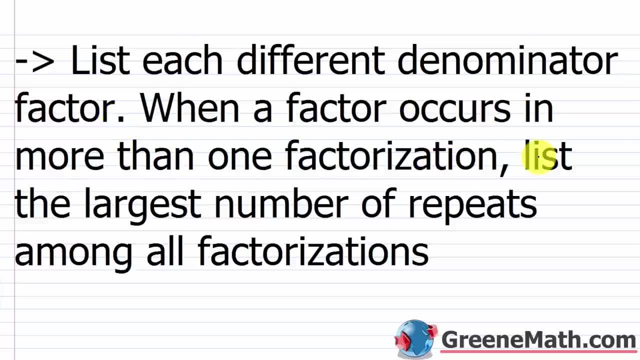 When a factor occurs in more than one factorization, list the largest number of repeats, okay, there it goes again, among all factorizations. 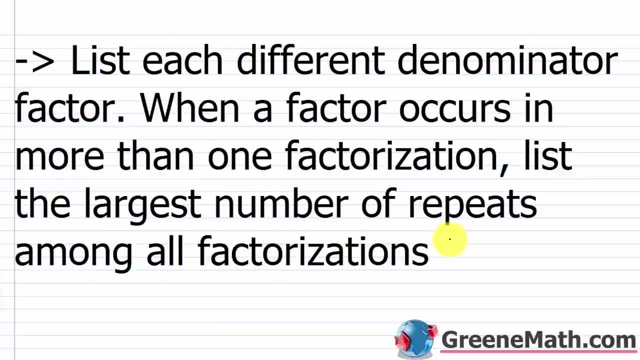 So again, this is the same process that we use when we're thinking about numbers. 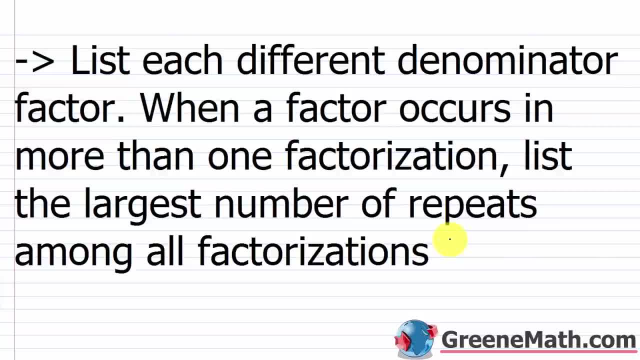 If I have a prime factor of 2 in one prime factorization and a prime factor of 2 in another one, I'm looking for the largest number of repeats between those two factorizations 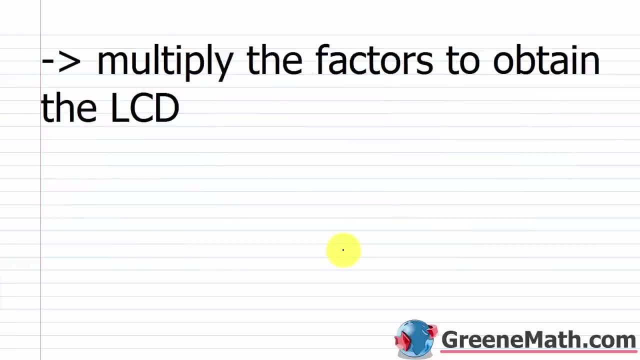 Alright, then the last step is just to multiply the factors to obtain the LCD. So again, same process as when we work with fractions, 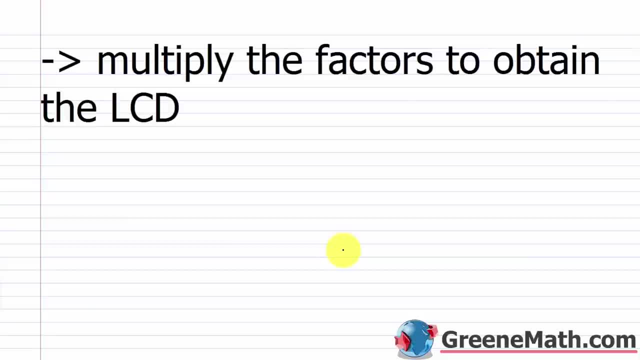 but it's just going to be a little bit more messy, a little bit more time consuming, a little bit more tedious, for the simple fact that we have variables involved. 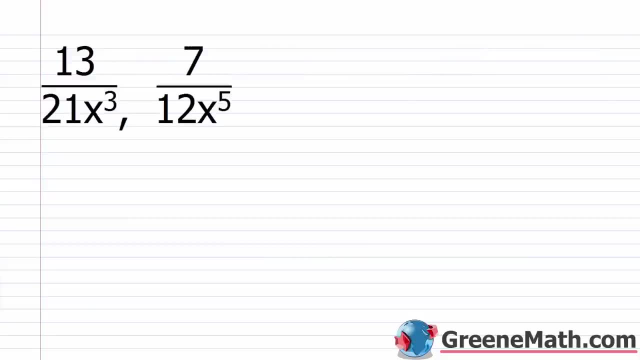 Alright, so let's start out with these two rational expressions. We have 13 over 21x cubed and we have 7 over 12x to the fifth power. So I just want to find the LCD. 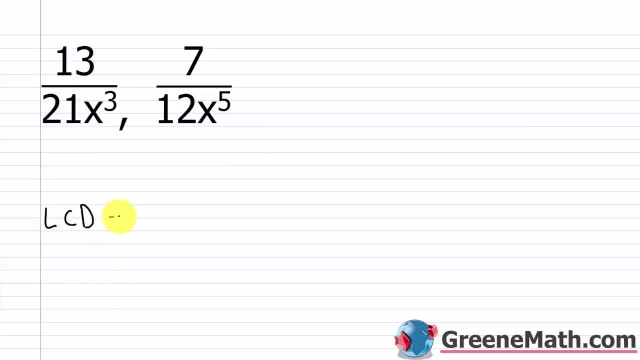 So I'm working with the denominators. So the LCD is what? It's the LCM of 21x cubed 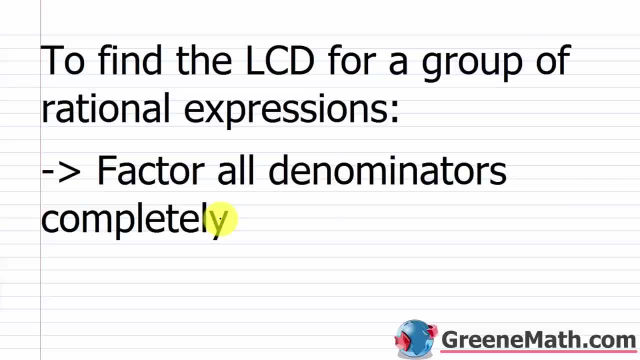 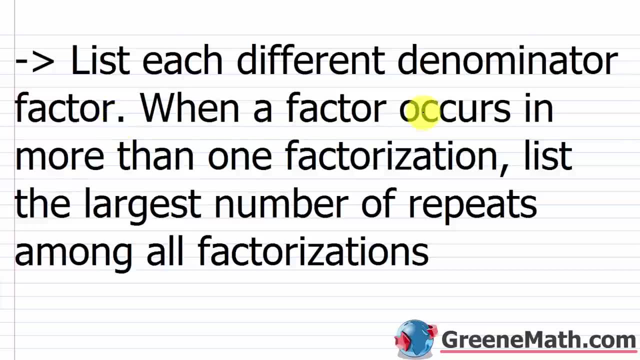 for the LCD, for a group of numbers, I'm going to factor the denominator. So I'm going to factor the denominators completely. I'm getting it down to the prime factorization of each number. Then I'm going to list each different denominator factor When a factor occurs in more than one factorization. 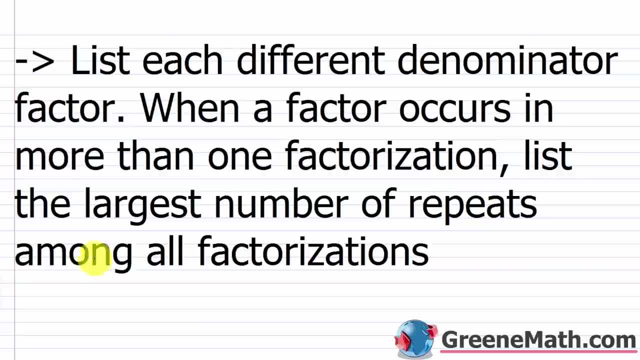 list the largest number of repeats. okay, there it goes again, among all factorizations. So again, this is the same process that we use when we're thinking about numbers. If I have a prime factor of two in one prime factorization and a prime factor of two in another one I'm looking for. 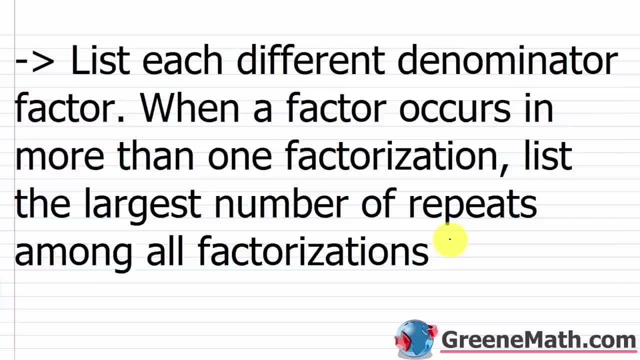 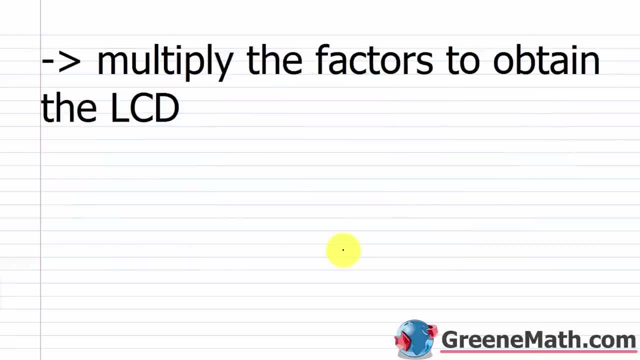 the largest number of repeats between the two. So I'm going to list the largest number of repeats between those two factorizations to put that in when I build my list. All right, then the last step is just to multiply the factors to obtain the LCD. So again same process as when we work with. 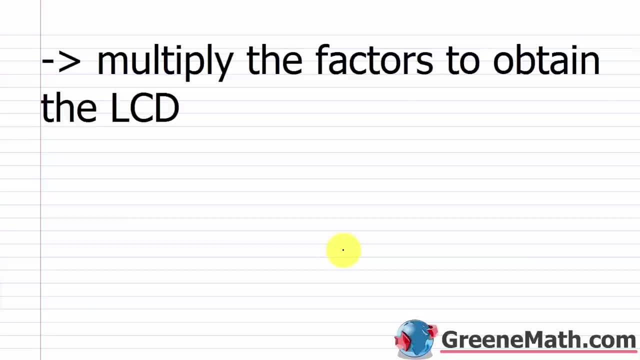 fractions, but it's just going to be a little bit more messy, a little bit more time consuming, a little bit more tedious, for the simple fact that we have variables involved. All right, so let's start out with these two rational expressions. We have 13 over 21x cubed. 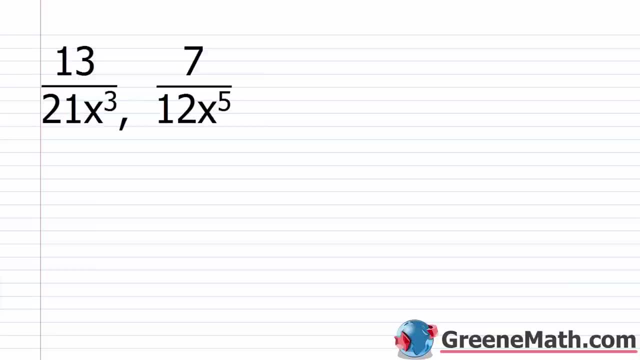 and we have 7 over 12x to the fifth power. So I just want to find the LCD. So I'm working with the denominators. So the LCD is what It's: the LCM of 21x cubed and of 12x to the fifth power. 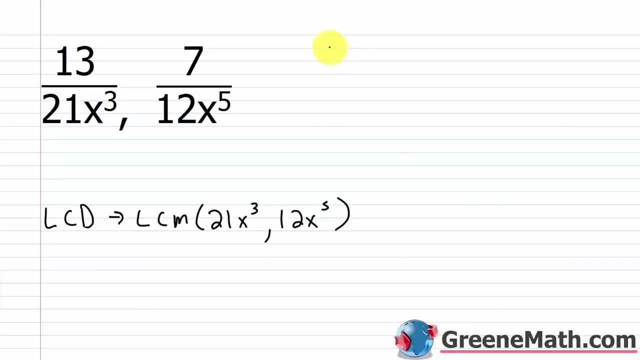 So pretty easy for the number parts. We already know how to do that right. We would just say: well, 21 is what It's 3 times 7, and 12 is 4 times 3.. 4 is 2 times 2.. 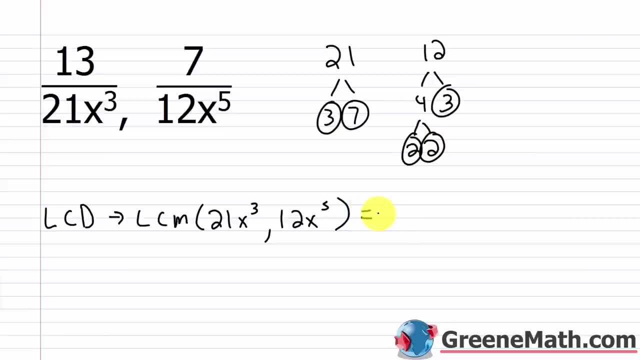 To build the number part. what would I do? I list every prime factor. I just watch out for duplicates. If I have a duplicate prime factor, meaning it occurs in more than one prime factorization, I'm looking for the largest number of repeats. So I have a 3 here and here It occurs. 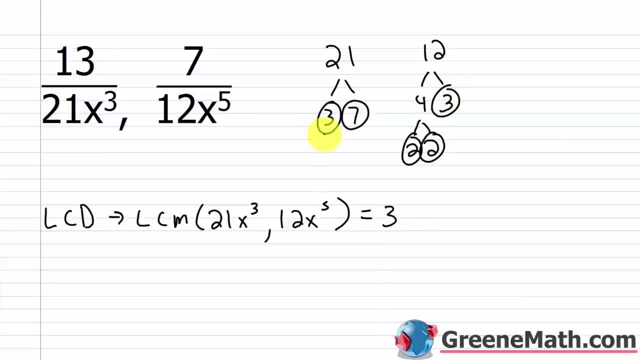 only once in each, so I'm just going to put 1 in here, not 2.. I have a 7 here, no 7 over here. I have two 2s in here, so I'm going to throw both of those in there and we know that's 4.. 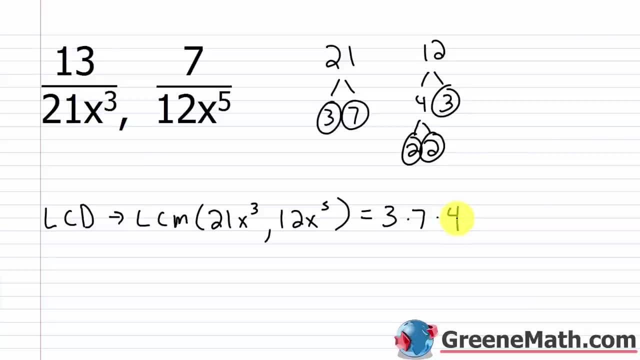 It's 3 times 7,, which is 21,, times 4,, which is 84.. So let's just go ahead and write 84 there. And then, what about the variable part? Well, do I really need to go through and say well? 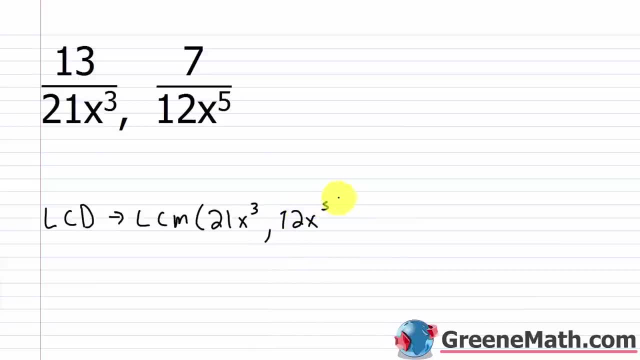 and of 12x to the fifth power. 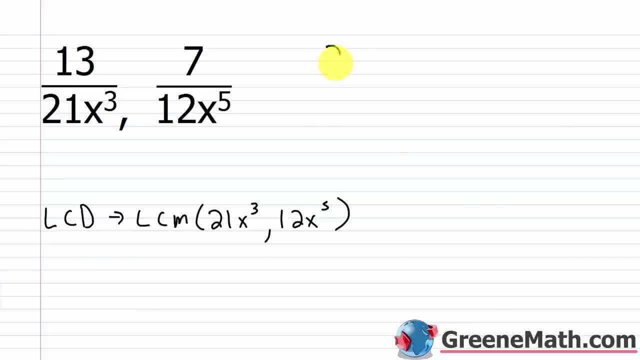 So pretty easy for the number parts. We already know how to do that, right? We would just say, okay, well, 1 is what? 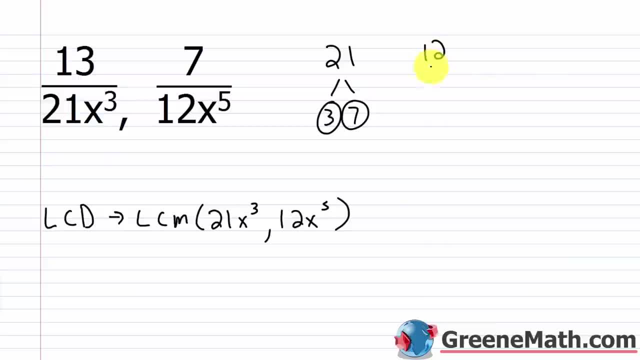 It's 3x7 and 12 is 4x3. 4 is 2x2. 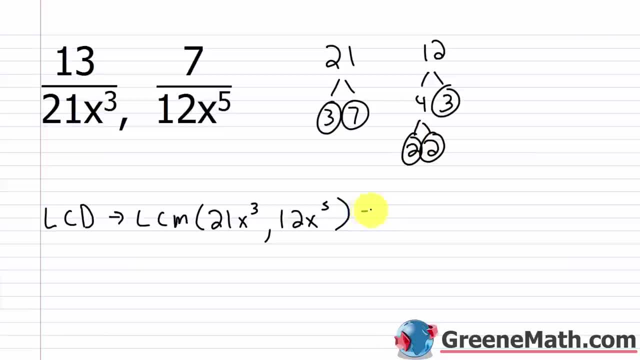 Alright, so to build the number part, what would I do? I list every prime factor. I just watch out for duplicates. If I have a duplicate prime factor, meaning it occurs in more than one prime factorization, I'm looking for the largest number of repeats. So I have a 3 here and here. It occurs only once in each, so I'm just going to put 1 in here. Not 2. I have a 7 here. No 7 over here. 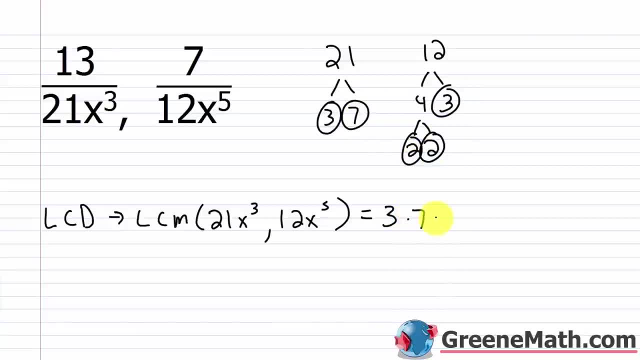 I have two 2s in here, so I'm going to throw both of those in there. And we know that's 4. 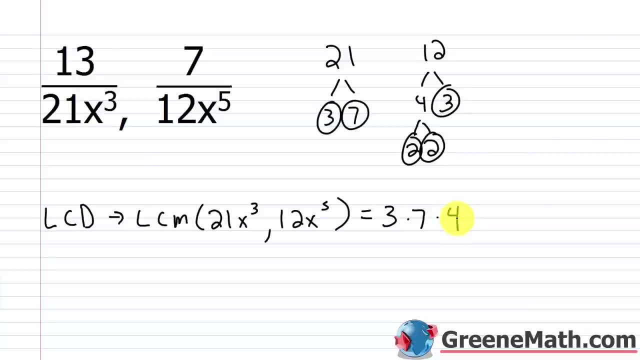 So the number part is 3x7, which is 21, times 4, which is 84. 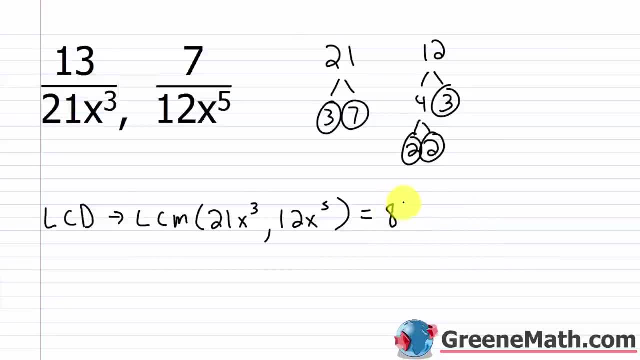 So let's just go ahead and write 84 there. And then what about the variable part? Well, do I really need to go through and say, well, I have x times x times x, and then I have x times x times x times x, and then I have x times x times x times x. Again, I want the largest number of repeats. So if it's the same variable, now I'm just going to go with the largest exponent. 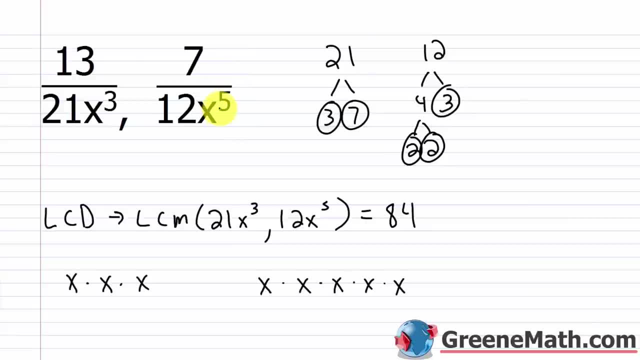 Remember, when we talked about the greatest common factor, we went with the smallest exponent. Now we're going with the largest exponent. So the largest exponent is the 5, so it's going to be 84x to the 5th power. That constitutes the largest number of repeats for either of the prime factorizations. So your LCD here is 84x to the 5th power. All right, let's take a look at another one. 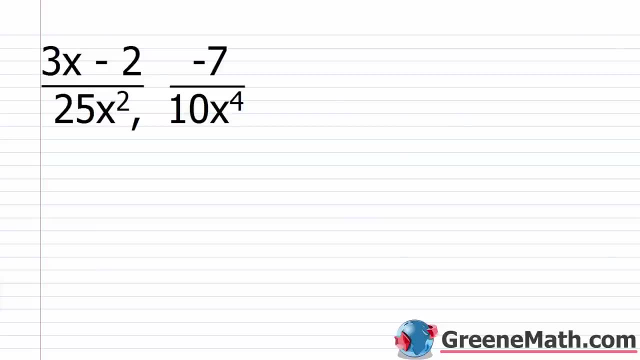 So we have 3x minus 2 over 25x squared, and then we also are looking at negative 7 over 10x to the 4th power. 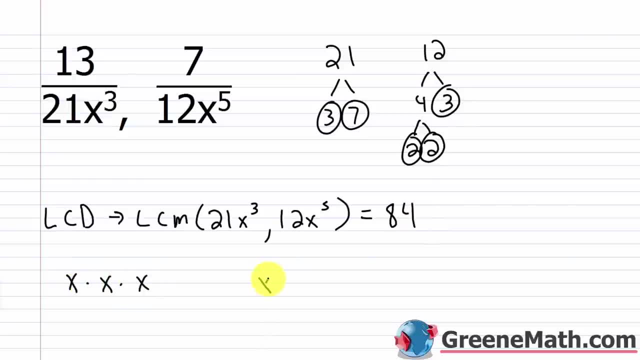 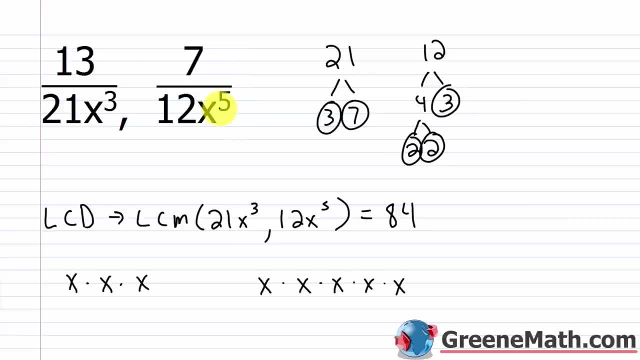 greatest common factor. we went with the smallest exponent. Now we're going with the largest exponent. So the largest exponent is the 5, so it's going to be 84x to the 5th power. That constitutes the largest number of repeats for either of the prime factorizations. So your LCD here is 84x to the 5th. 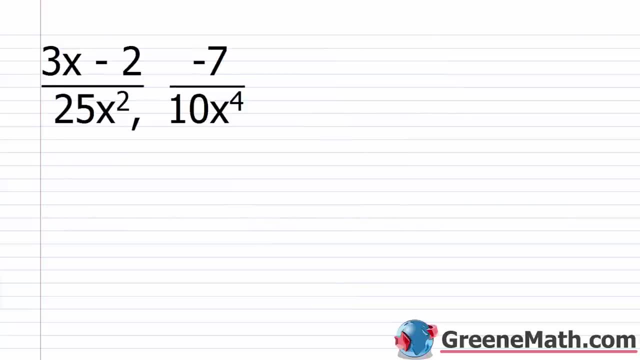 power. All right, let's take a look at another one. So we have 3x minus 2 over 25x squared, and then we also are looking at negative 7 over 10x to the 4th power. LCD by LCD is the LCM of these two denominators. So 25x squared and then 10x to the 4th power. 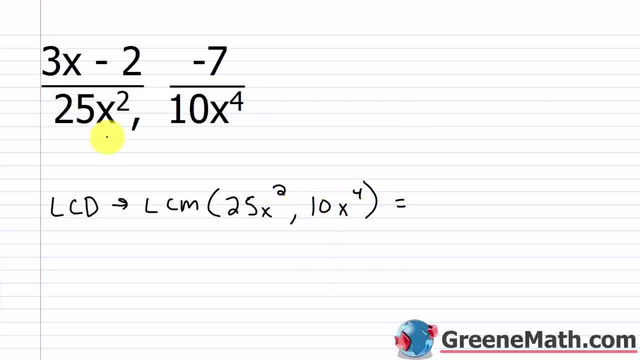 So again, we know how to do the number part. We can almost do that in our head. We know 25 is what It's 5 times 5, and 10 is 5 times 2.. So I know that I have a duplicate prime factor of 5. It occurs twice here. 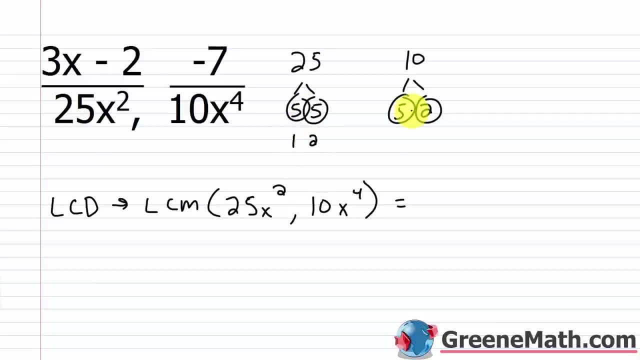 so 1 and then 2.. Two factors of 5 here, only 1 here. So I go with the largest number of repeats, and that's in the prime factorization of 25.. So I'm going to throw two of those in here 5 times. 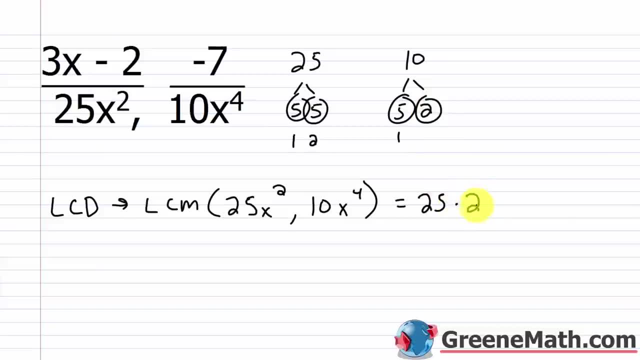 5 is 25, and then I'm going to throw a 2 in there. So times 2, 25, times 2 is 50. So the number part is a 50.. Now for the variable part. I have x squared and I have x to the 4th power. 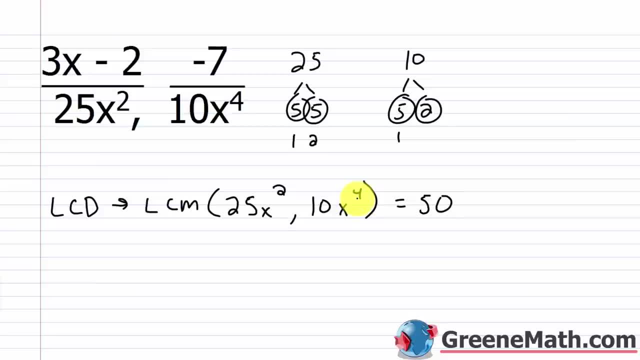 Again, I want to go with the largest exponent on x, and the reason for that is that's going to be the largest number of repeats between the two prime factorizations. If I had x squared, it's x times x, so 2 of those. If I have x to the 4th power, I have x times x times x times x. This is: 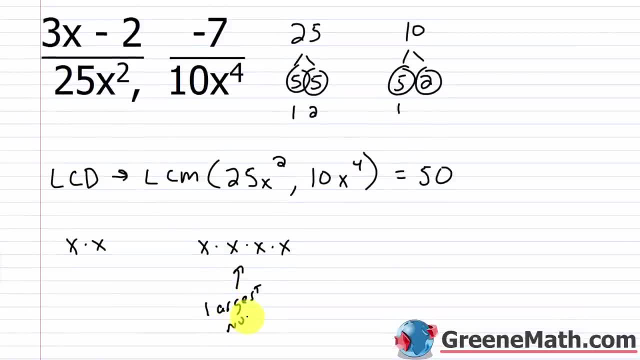 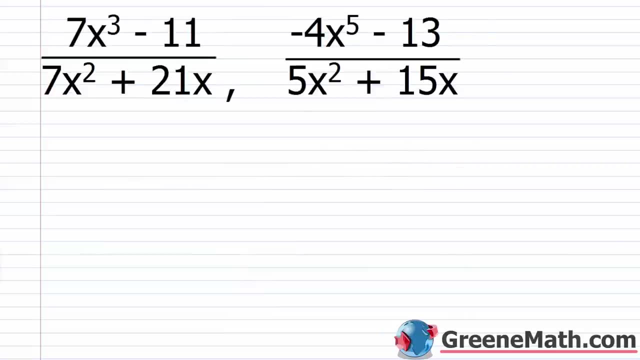 the largest number. This is the largest number again, as given by the largest exponent, So I just use that. So this is 50x to the 4th power. All right, so let's take a look at a number. 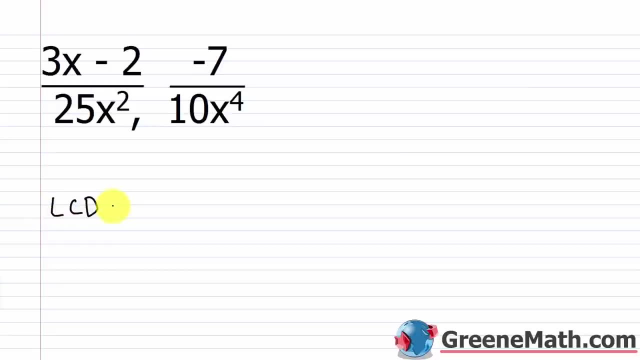 So again, my LCD is the LCM of these two denominators, so 25x squared and then 10x to the 4th power. 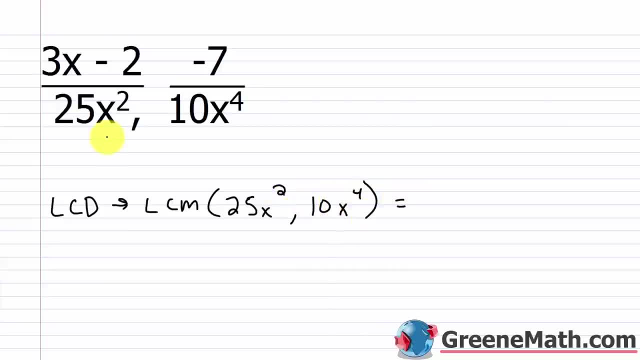 So again, we know how to do the number part. We can almost do that in our head. So 25 is what? It's 5 times 5, and 10 is 5 times 2. 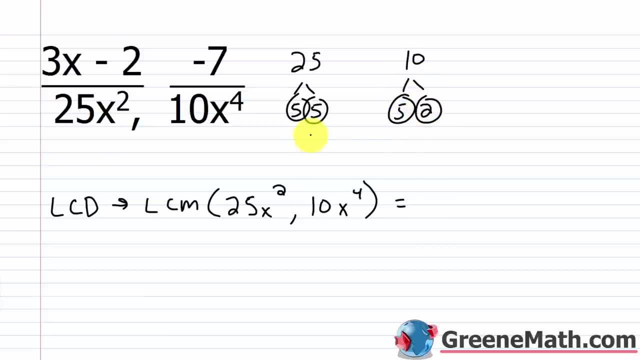 So I know that I have a duplicate prime factor of 5. It occurs twice here, so 1 and then 2. Two factors of 5 here, only one here. So I go with the largest number of repeats, and that's in the prime factorization of 25. So I'm going to throw two of those in here. 5 times 5 is 25. And then I'm going to throw a 2 in there. 25 times 2. 25 times 2 is 50. So the number part is a 50. 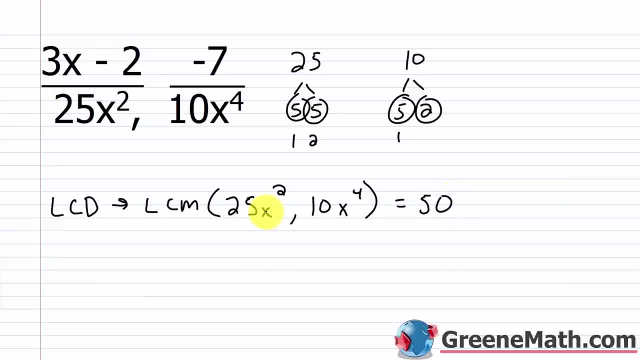 Now for the variable part, I have x squared and I have x to the 4th power. Again, I want to go with the largest exponent on x, and the reason for that is, that's going to be the largest number of repeats between the two prime factorizations. 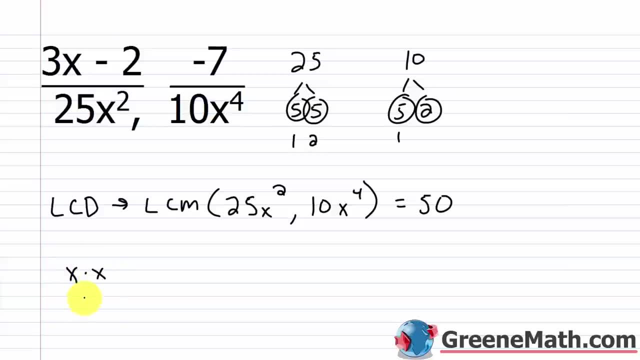 If I had x squared, it's x times x, so two of those. 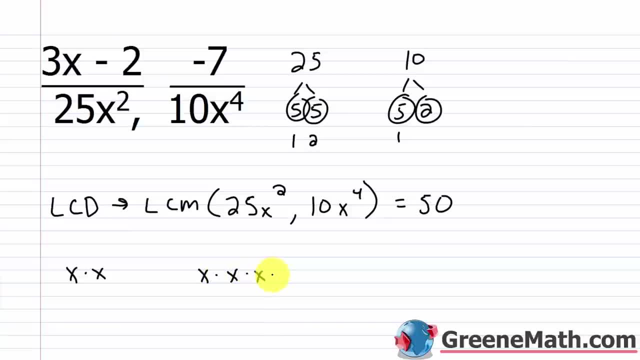 If I have x to the 4th power, I have x times x times x times x. This is the largest number. This is the largest... 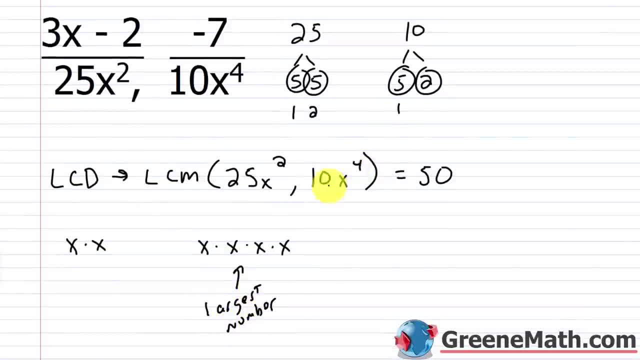 number, again, as given by the largest exponent. So I just use that. So this is 50x to the 4th power. Alright, so let's take a look at another one. 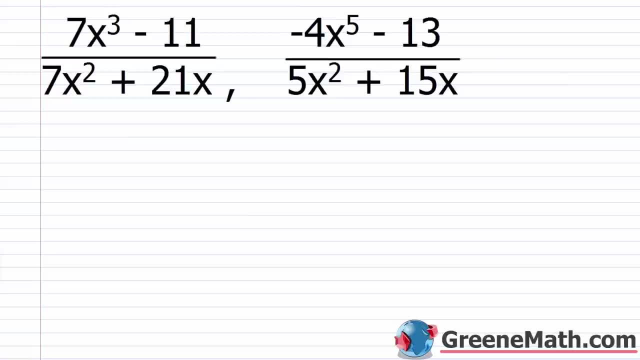 We have 7x cubed minus 11, over 7x squared plus 21x, and then we have negative 4x to the 5th power minus 13, over 5x squared plus 15x. 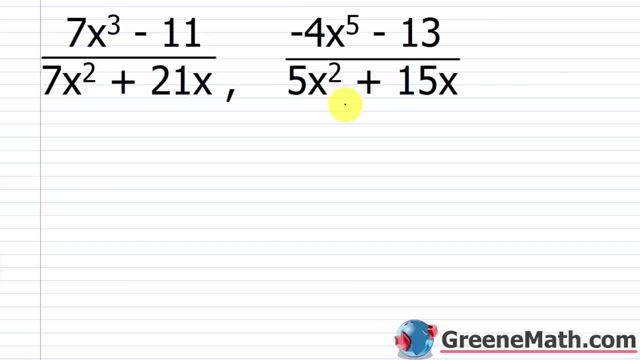 Now, for this one, you might start thinking about, and this is really complicated, what do we do? 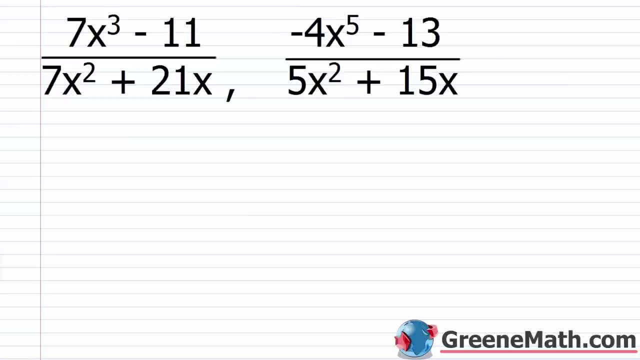 We have 7x cubed minus 11 over 7x, squared plus 21x. and then we have negative x squared minus negative 4x to the 5th power, minus 13 over 5x squared plus 15x. Now for this one, you might. 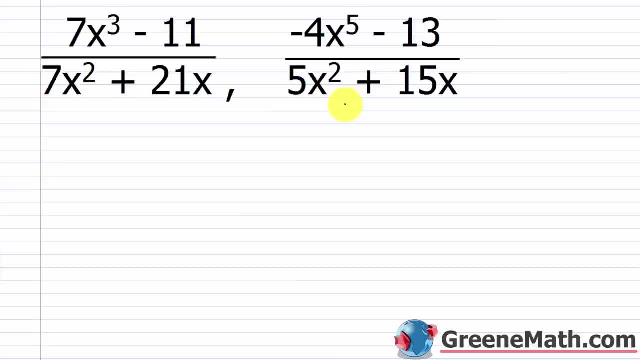 start thinking about: man, this is really complicated. What do we do? Again, you got to factor everything completely. So I want the LCD of these two guys. The first thing I'm going to do is I'm going to factor them. So from this first guy here I can pull out a 7x, So I can pull out. 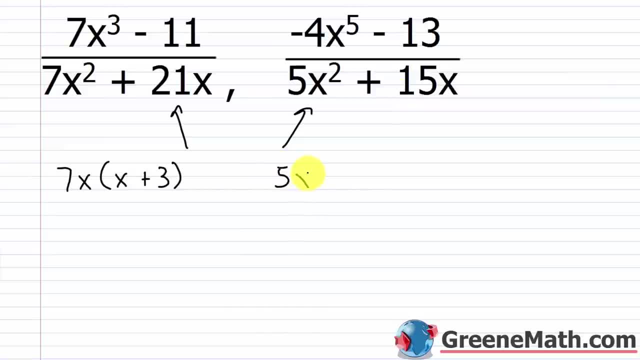 a 5x. So I pull out a 5x and what's left is x plus 3.. So now I'm looking at what's common. So I have x plus 3, and I have x plus 3.. So when I build my LCD, my LCD, I'm going to have a factor 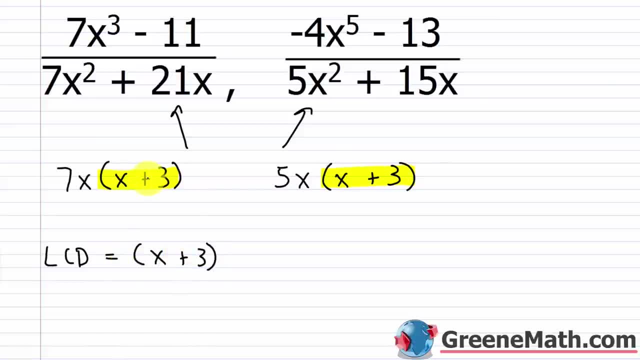 of x plus 3 in there. It occurs only once in each, so that's all I'm going to do Now. each one has an x. I have an x here and I have an x In each case. it's only one, So I'm going to put one x in. 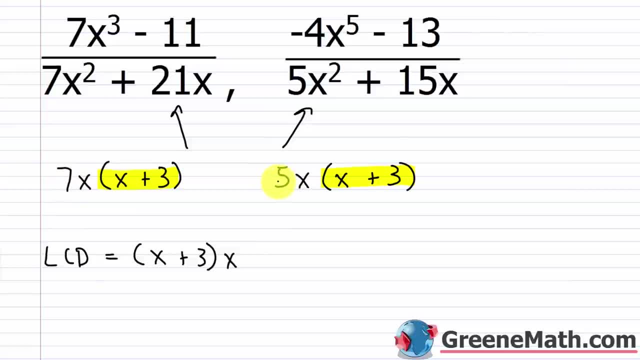 there, and then I have a 7, and I have a 5.. So I'm going to put one x in there and then I have a 5.. Each of those is a prime number. 7 times 5 is 35. So what this is going to be, it's going to be: 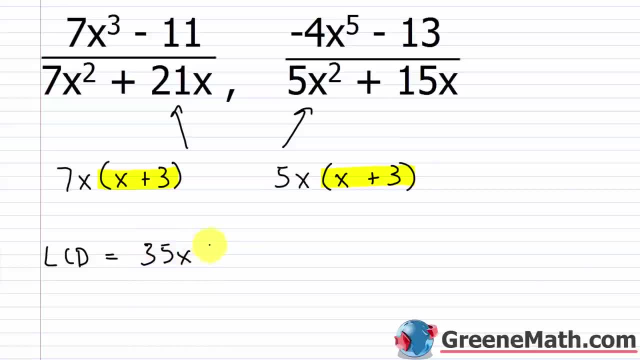 35x times x plus 3, that quantity, And I would just leave it just like this, in factored form. You can go through and multiply it if you want, but usually when you're finding an LCD it's just better to leave it in factored form in case you need to do some canceling later on. All right, 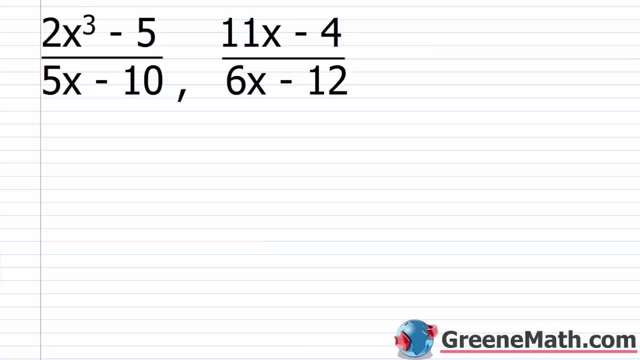 let's take a look at another one. So we have 2x cubed minus 5 over 5x minus 10.. Then we have 11x minus 4 over 6x minus 12.. So again, I want to look at these two denominators and I want to factor them completely. 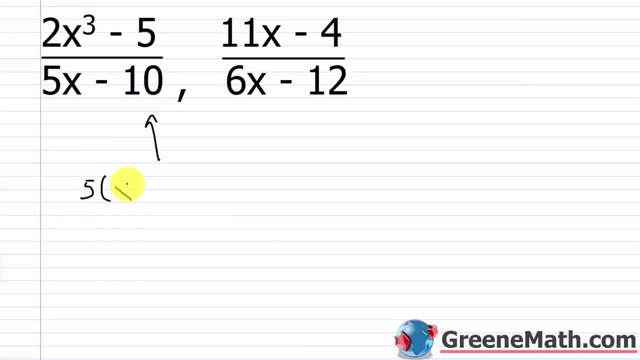 So for this one, I could pull out a 5, and I would have x minus 2.. For this one, I could pull out a 6, and I would have x minus 2.. So you can see, you have x minus 2 and x minus 2.. 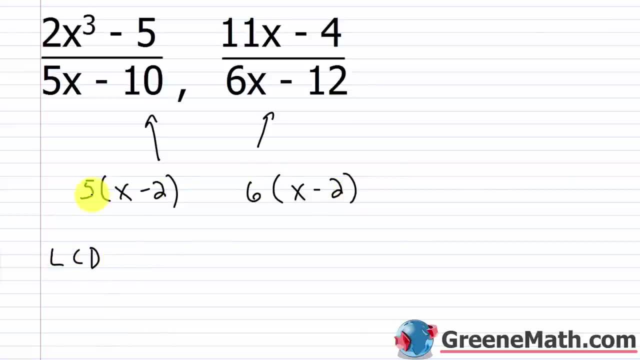 So for the LCD, you're going to have what You have: a 5 and you have a 6.. 5 times 6 is going to be what, That's going to be 30. And then you have that x minus 2.. 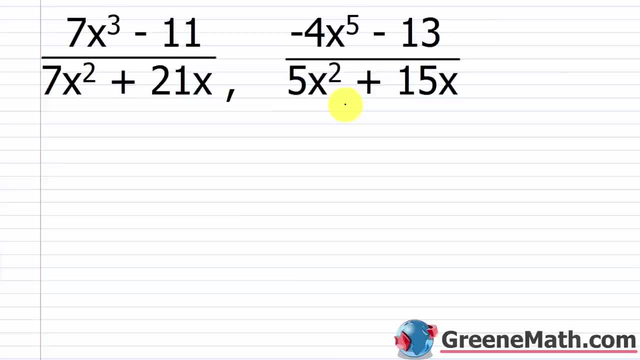 Again, you've got to factor everything completely. So I want the LCD of these two guys. The first thing I'm going to do is I'm going to factor them. So from this first guy here, I can pull out a 7x. 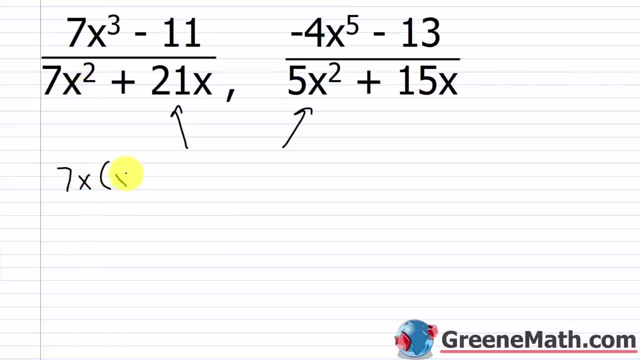 So I can pull out a 7x, and then what's left inside is x plus 3. From this guy right here, I can pull out a 5x. 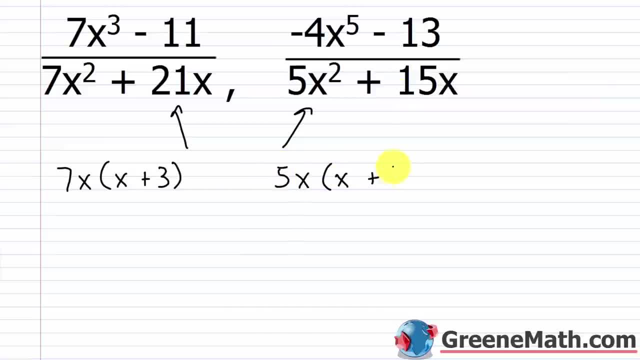 So I pull out a 5x, and what's left is x plus 3. 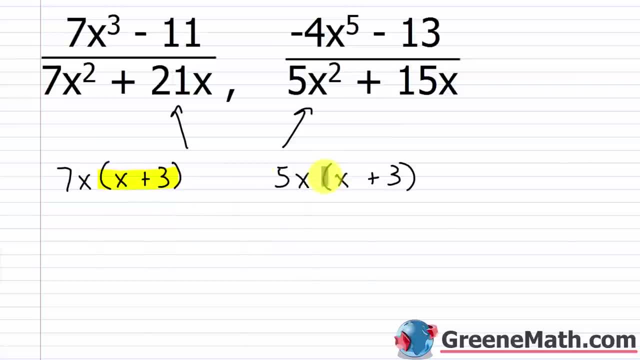 So now I'm looking at what's common. So I have x plus 3, and I have x plus 3. 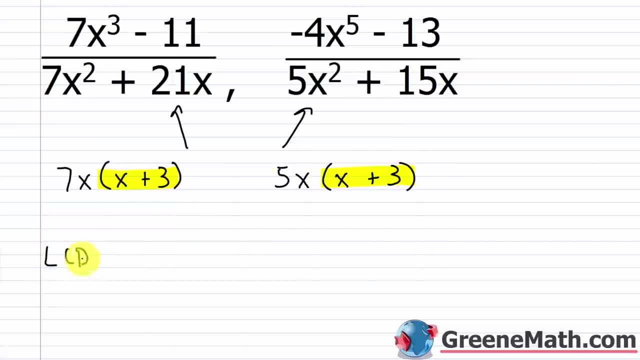 So when I build my LCD, my LCD, I'm going to have a factor of x plus 3 in there. It occurs only once in each, so that's all I'm going to do. 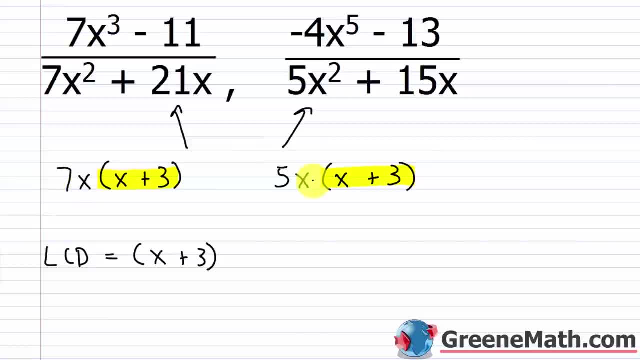 Now, each one has an x. I have an x here, and I have an x. In each case, it's only one. So I'm going to put one x in there, and then I have a 7, and I have a 5. Each of those is a prime number. 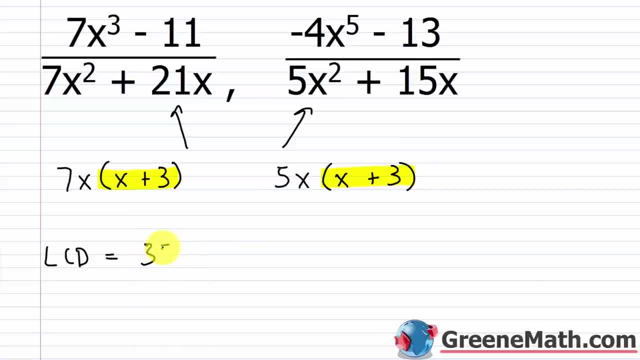 So what this is going to be, it's going to be 35x, 35x times x plus 3, that quantity. 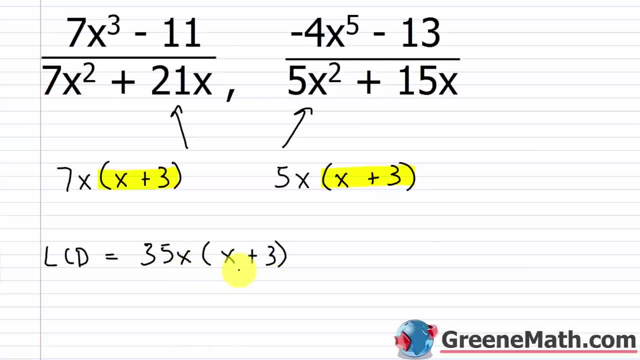 So I would just leave it just like this in factored form. You can go through and multiply it if you want, but usually when you're finding an LCD, it's just better to leave it in factored form in case you need to do some canceling later on. 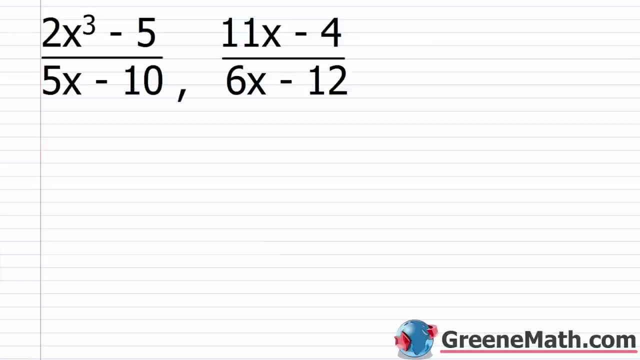 All right, let's take a look at another one. So we have 2x cubed minus 5 over 5x minus 10. Then we have 11x minus 4 over 6x minus 12. So again, I want to look at these two denominators, and I want to factor them completely. So for this one, I could pull out a 5, and I would have x minus 2. 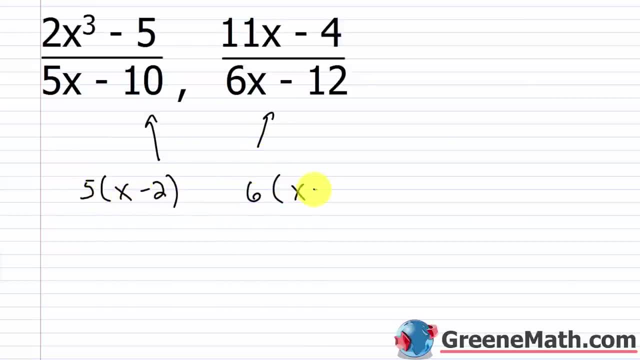 For this one, I could pull out a 6, and I would have x minus 2. So you can see you have x minus 2 and x minus 2. 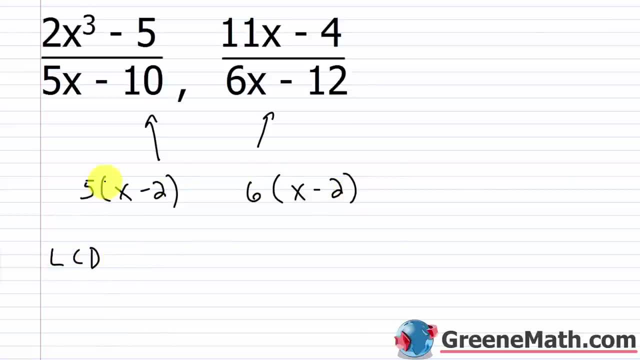 So for the LCD, you're going to have what? You have a 5 and you have a 6. 5 times 6 is going to be what? That's going to be 30. And then you have that x minus 2. 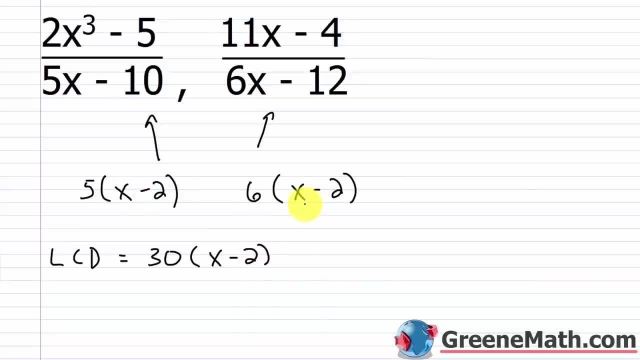 It only occurs once in each factorization, so that's all I need to do when I put it in here. I've got one factor of x minus 2, then I've got one factor of 5, and one factor of 6, because 6 is 2 times 3 and 5 is prime. So 5 times 2 times 3 would give me 30. That's how I got that. And then I've got my one factor of x minus 2. 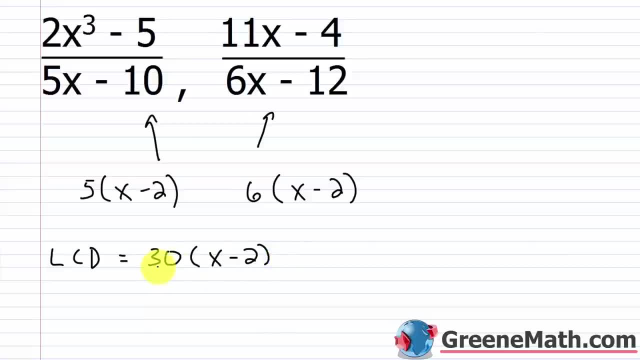 So you get 30 times the quantity x minus 2. And again, I would leave this in factored form. 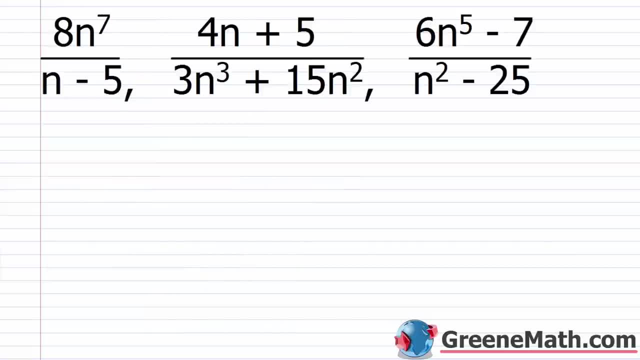 All right, let's take a look at one more problem. I think you get the general idea. So we have n minus 5. I can't really factor that. I'll just write n minus 5. 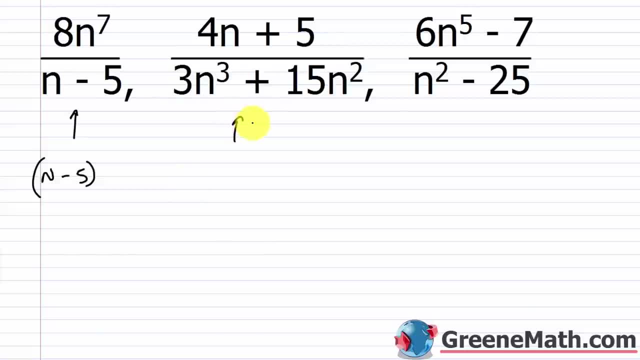 I have 3n cubed plus 15n squared. So I could pull out a 3n squared, and I would get n plus 5. 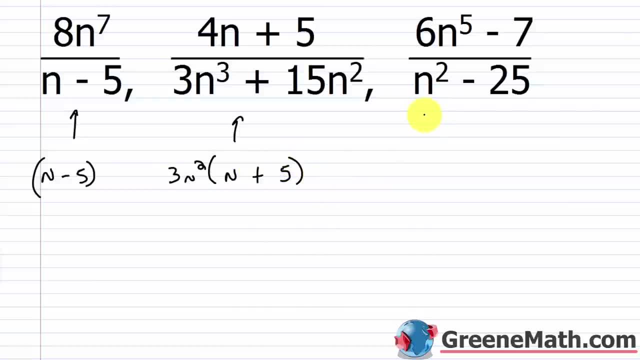 And then over here, I have n squared minus 25. That's the difference of two squares. So this is n minus 5 times n plus 5. 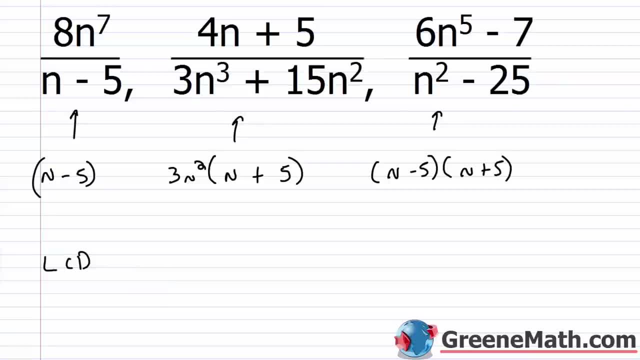 So for my LCD, what do I have? I have n minus 5 here and also here. And then I have n plus 5 here and also here. So each only occurs once. This occurs once. This occurs twice. This occurs once. So I would just put 1 in there. And then this occurs once, and this occurs once. So I would just put 1 in there. 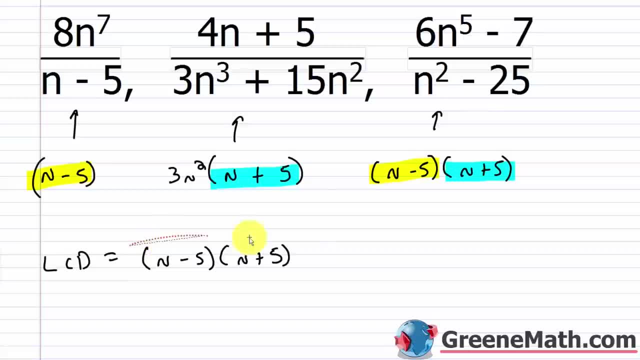 And then we have this 3n squared that's got to go in. So let me kind of scooch this down. So we like it to be in the front. That's just more traditional. And so our LCD is 3n squared times the quantity n minus 5 times the quantity n plus 5. 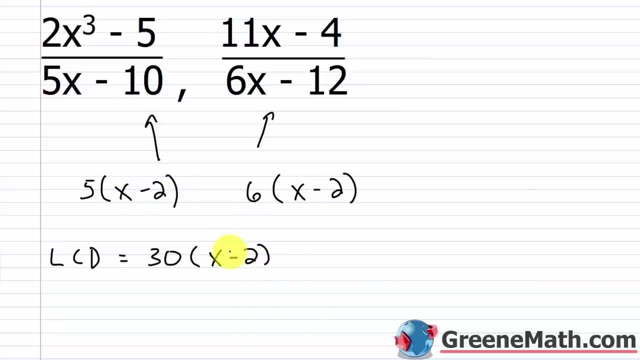 It only occurs once in each factorization, so that's all I need to do. when I put it in here, I've got one factor of x minus 2, and then I've got one factor of 5 and one factor of 6,. 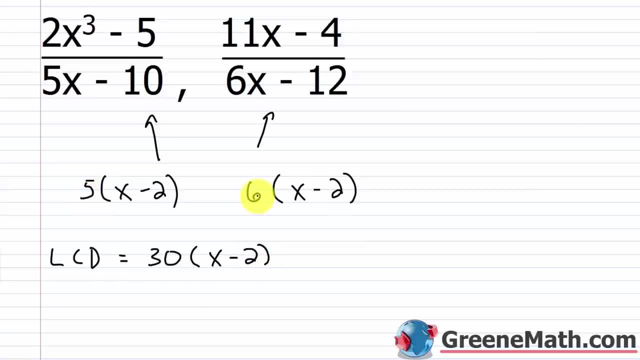 because 6 is 2 times 3 and 5 is prime. So 5 times 2 times 3 would give me 30. That's how I got that. And then I've got my one factor of x minus 2.. 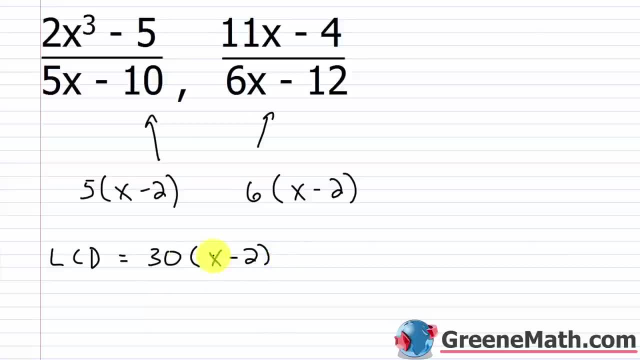 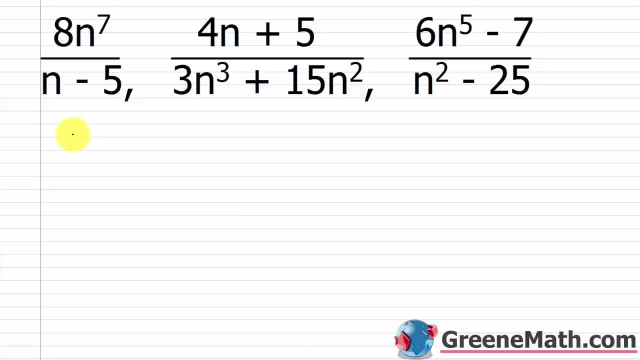 So you get 30 times the quantity x minus 2.. And again, I would leave this in factored form. All right, let's take a look at one more problem. I think you get the general idea. So we have n minus 5.. 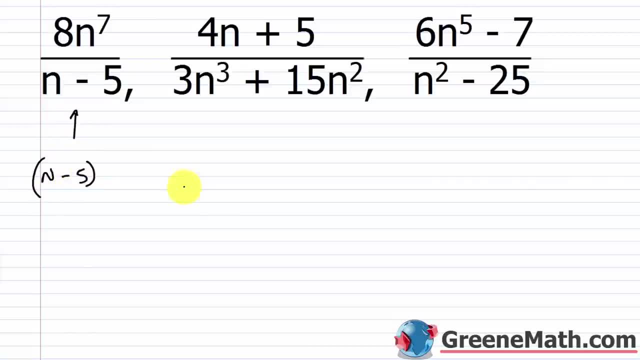 I can't really factor that. I'll just write n minus 5.. I have 3n cubed plus 15n squared, So I could pull out a 3n squared and I would get n plus 5.. And then over here I have n squared minus 25.. 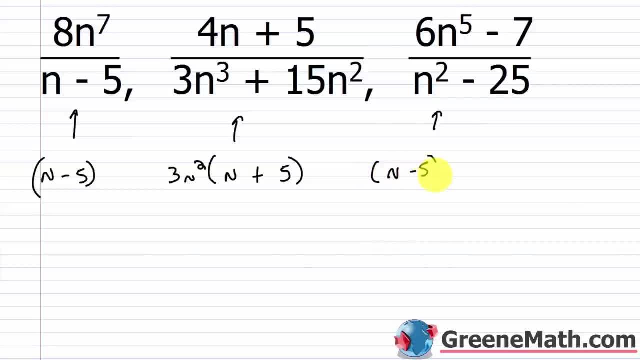 That's the difference of two squares. So this is n minus 5 times n plus 5.. So for my LCD, What do I have? I have n minus 5 here and also here, And then I have n plus 5 here and also here. 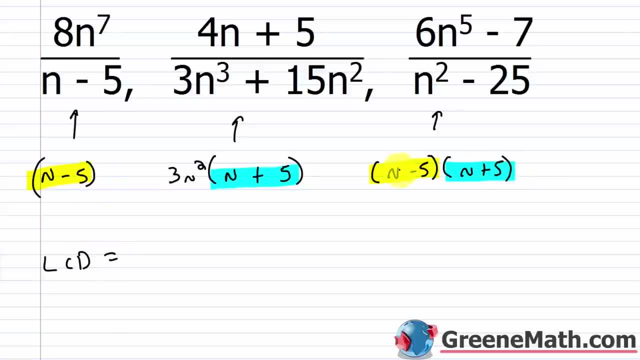 So each only occurs once. This occurs once, This occurs once, So I would just put one in there, And then this occurs once, and this occurs once, So I would just put one in there, And then we have this 3n squared. that's got to go in. 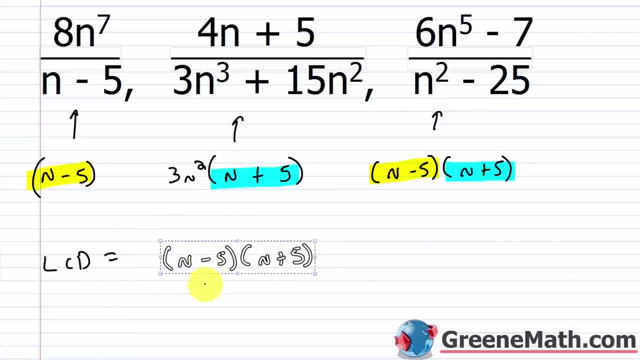 So let me kind of scooch this down. So we like it to be in the front. That's just more traditional. And so our LCD is 3n squared times the quantity n minus 5, times the quantity n plus 5.. 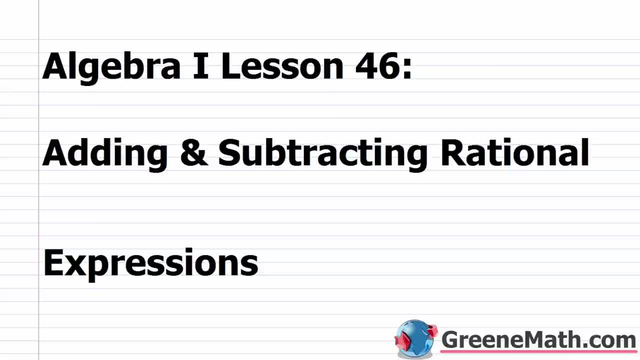 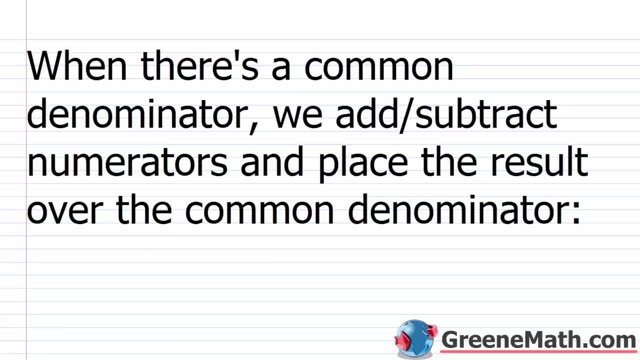 Hello and welcome to Algebra 1, Lesson 46.. In this video we're going to learn about adding and subtracting rational expressions. So when we're adding or subtracting rational expressions we need to first have a common denominator. It's just like when we added or subtracted fractions back in pre-algebra. 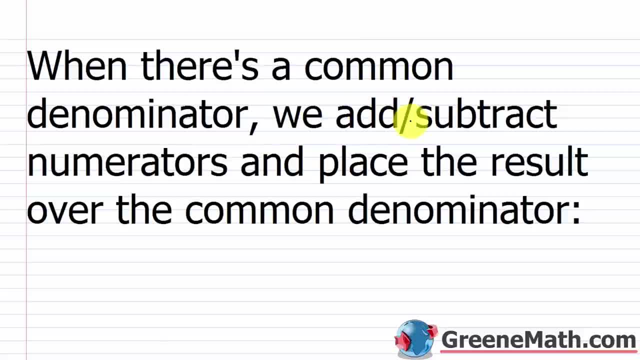 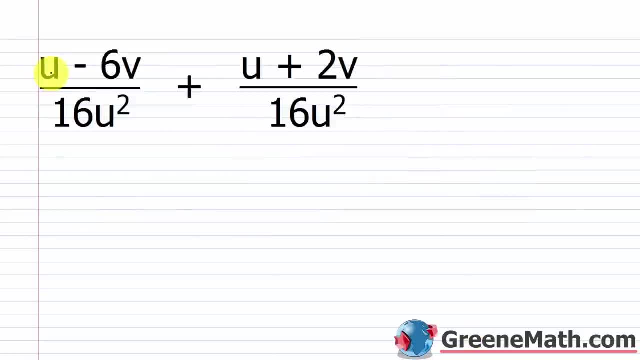 So when there's a common denominator, all we need to do is add or subtract the numerators and place the result over the common denominator. All right, for the first one we're going to look at, we have u minus 6v over 16u squared. 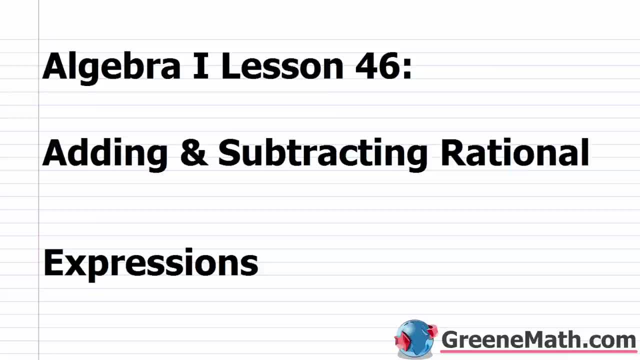 Hello, and welcome to Algebra 1 Lesson 46. In this video, we're going to learn about adding and subtracting rational expressions. 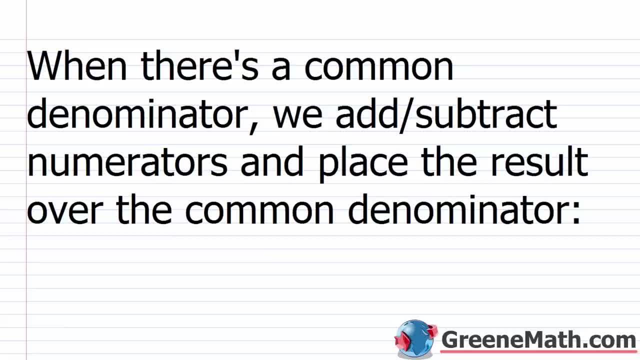 So when we're adding or subtracting rational expressions, we need to first have a common denominator. It's just like when we added or subtracted fractions back in pre-algebra. So when there's a common denominator, all we need to do is add or subtract the numerators and place the result over the common denominator. 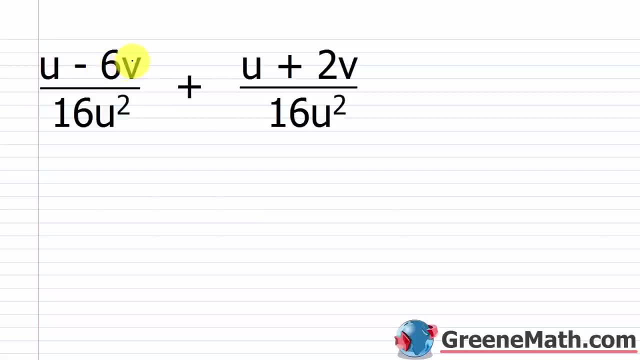 All right, for the first one we're going to look at, we have u minus 6v over 16u squared, then plus u plus 2v. Again, over 16u squared. So you can see that we have a common denominator of 16u squared. So just like with fractions, all we need to do is add the numerators and put the result over that common denominator. So just to show you real quick, it's the same thing as if I had something like, let's say, 1 fifth plus 2 fifths. 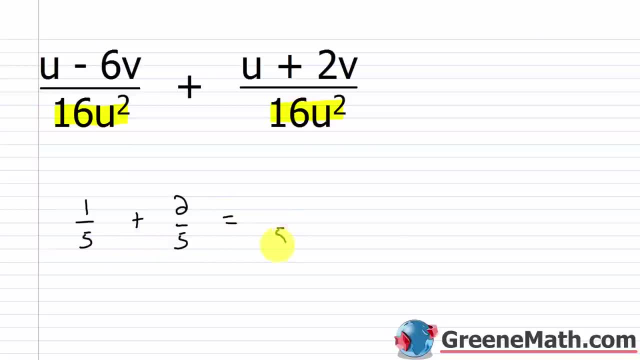 I have a common denominator of 5, so that just stays the same, and then I just add the numerators. 1 plus 2 is 3, and so I get 3 fifths. 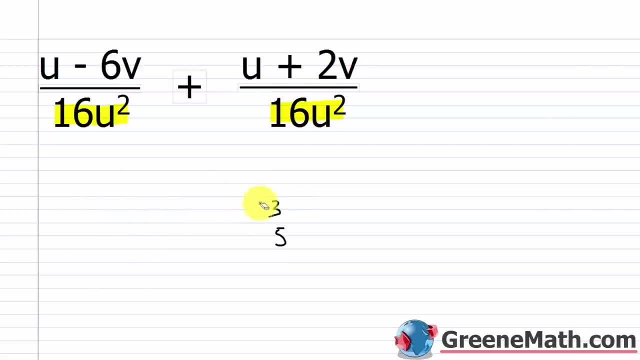 So here I'm going to do the exact same process. It's just going to be a little bit more tedious because I have some variables involved, right? It's just going to be more work. So I'm going to keep this part the same, 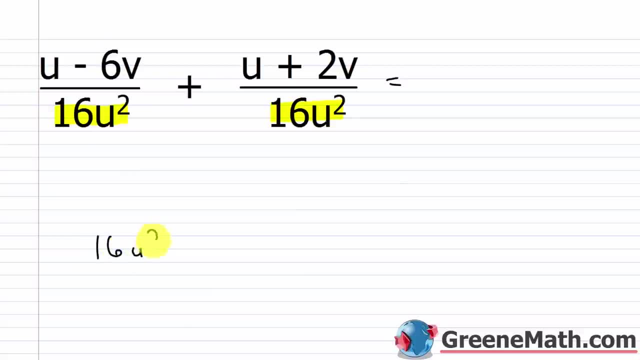 so 16u squared. That will remain unchanged. 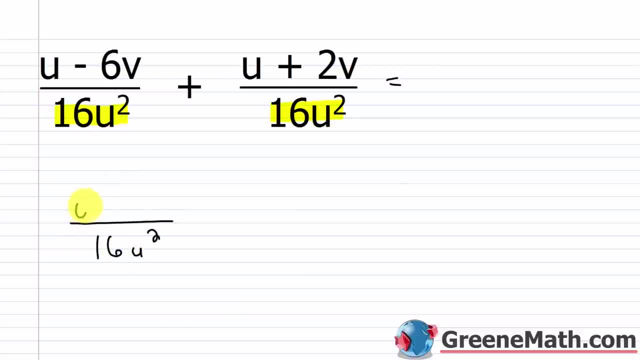 Then for the numerators, I have u minus 6v, so u minus 6v, then plus u plus 2v. Kind of expand this out a little bit. Let me write this in the center. 16u squared. 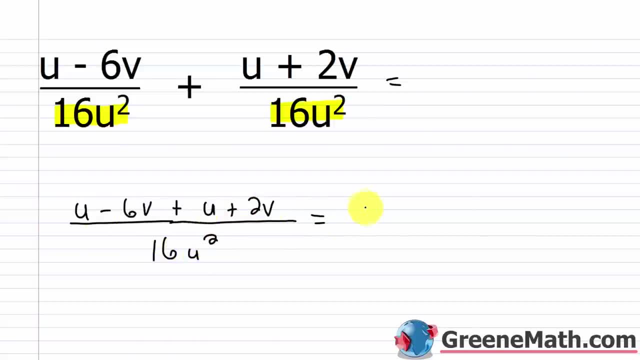 And I just want to combine like terms in the numerator. So u plus u is 2u, and then negative 6v plus 2v is going to be negative 4v. And again, this is over the common denominator 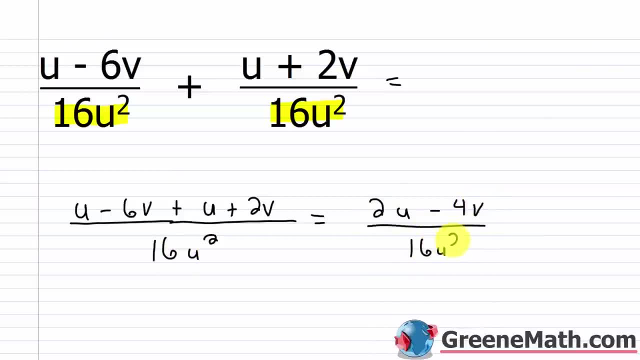 of 16u squared. Now in a lot of cases, you'll stop and you'll say, this is my answer. I'll box this up and say, I'm done. But there's a problem here. 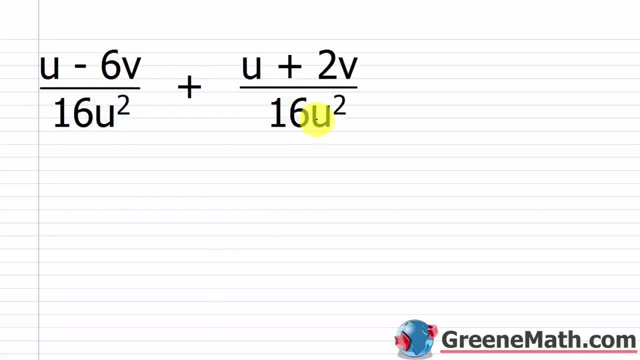 then plus u plus 2v, again over 16u squared. So you can see that we have a common denominator of 16u squared. So, just like with fractions, all we need to do is add the numerators and put the result over that common denominator. 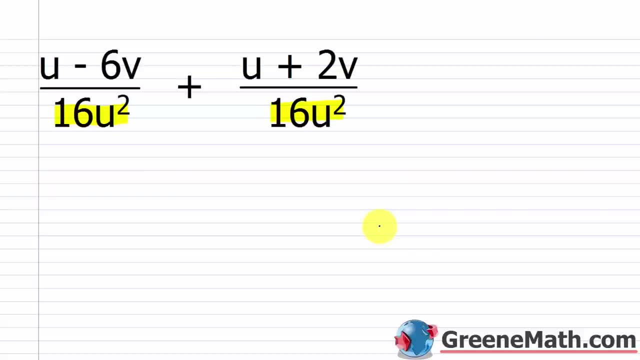 So just to show you real quick, it's the same thing as if I had something like, let's say, 1, 1⁄5 plus 2⁄5.. I have a common denominator of 5, so that just stays the same. 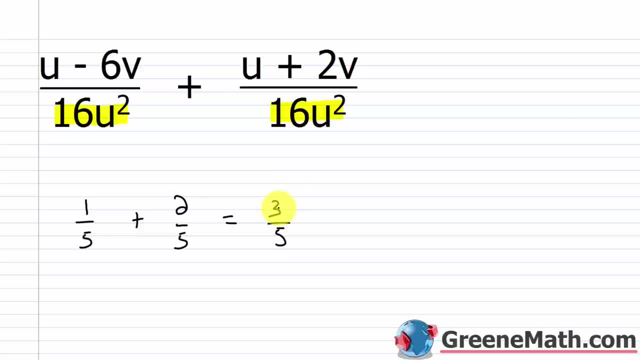 And then I just add the numerators: 1 plus 2 is 3, and so I get 3⁄5.. So here I'm going to do the exact same process. It's just going to be a little bit more tedious. 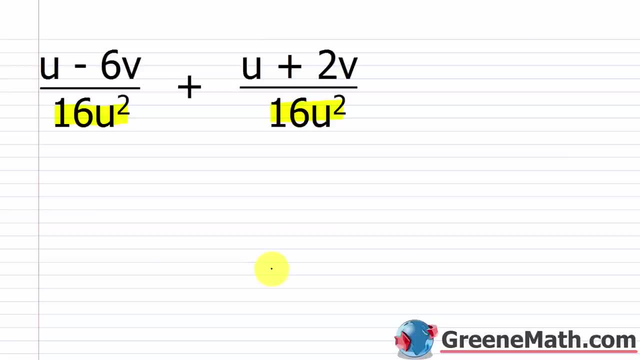 because I have some variables involved. right, It's just going to be more work, So I'm going to keep this part the same. So 16u squared, that will remain unchanged. Then for the numerators, I have u minus 6v. 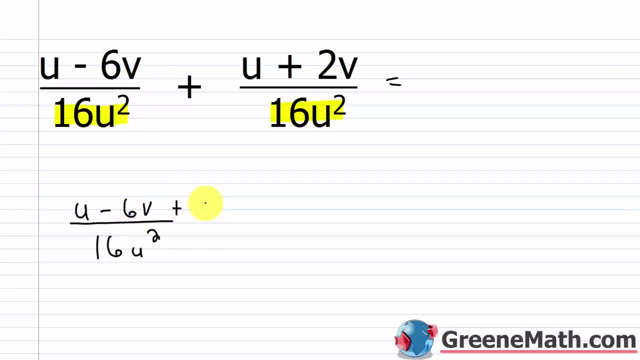 So u minus 6v, then plus u plus 2v. Kind of expand this out a little bit. We'll write this in the center, 16u squared, And I just want to combine like terms in the numerator. So u plus u is 2u. 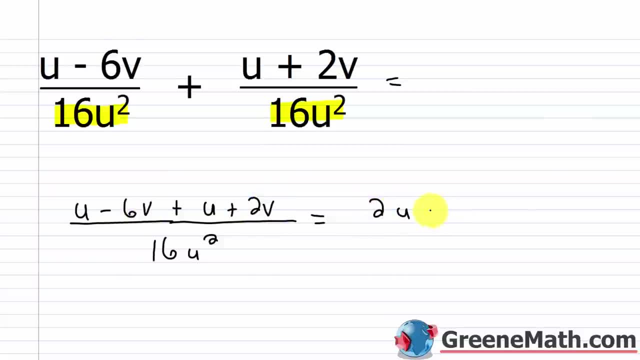 And then negative 6v plus 2v is going to be negative 4v And again this is over the common denominator of 16u squared. Now, in a lot of cases you'll stop and you'll say: this is my answer, right. 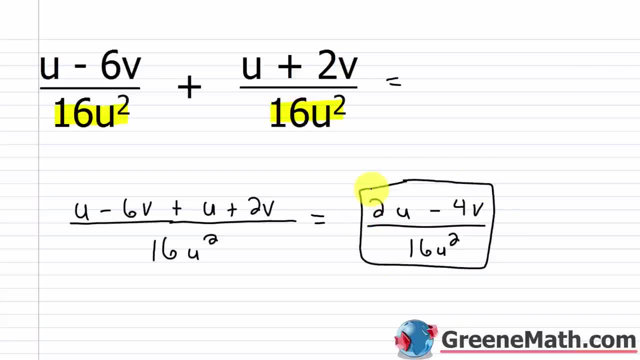 I'll box this up and say I'm done. But there's a problem here. Remember, when we report our answer with fractions, we want to see if we can reduce the fraction to its lowest terms right, Or simplify it. You're always expected to do that. 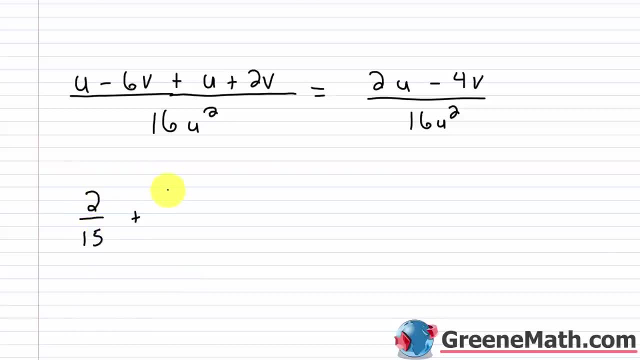 If I had something like 2 15ths plus 3 15ths and that common denominator of 15, 2 plus 3 is 5.. Now I wouldn't leave my answer this way. I would say: okay, the greatest common factor. 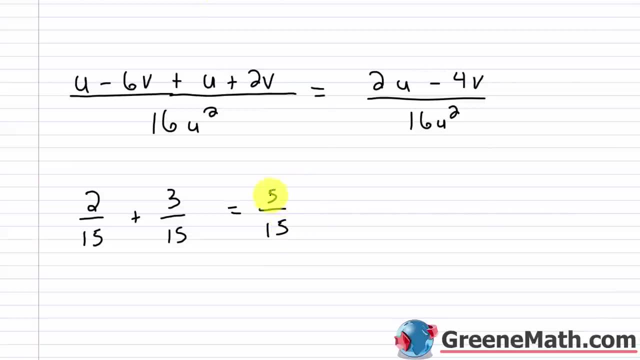 between these two is 5.. So I would divide the numerator by 5 and I would get 1.. I would also divide the denominator by 5 and I get 3.. And so my simplified answer here is: 1- 3rd. 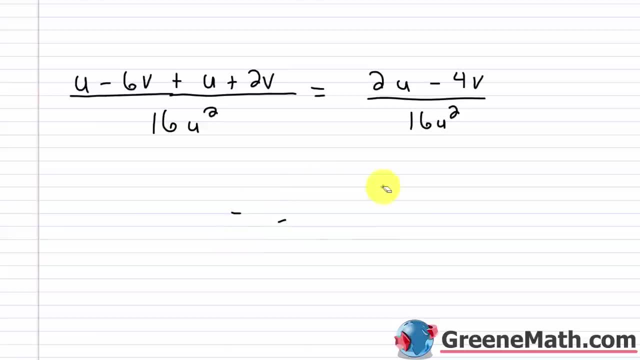 So I'm going to do the same thing here, And all I really need to do is just factor it to see what the GCF would be. So in the numerator I can pull out a 2.. So this would be 2 times the quantity u minus 2v. 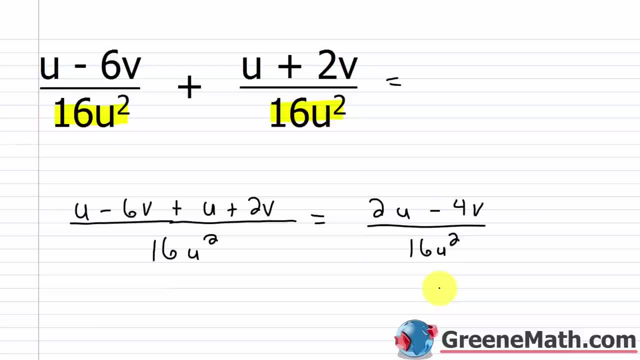 Remember, when we report our answer with fractions, we want to see if we can reduce the fraction to its lowest terms, right? Or simplify it. You're always expected to do that. 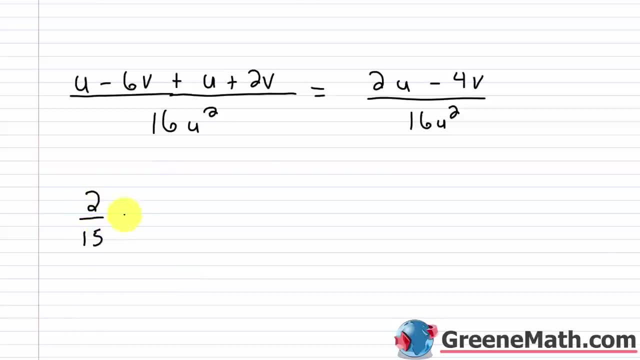 If I had something like 2 15ths plus 3 15ths and that common denominator of 15, 2 plus 3 is 5. 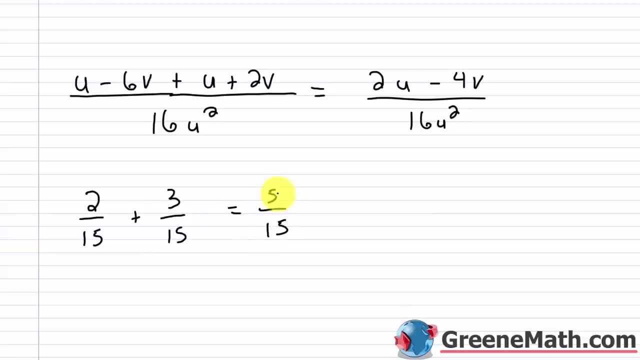 Now I wouldn't leave my answer this way. I would say, okay, the greatest common factor between these two is 5. So I would divide the numerator by 5 and I would get 1. I would also divide the denominator by 5 and I get 3. And so my simplified answer here is 1 3rd. So I'm going to do the same thing here. 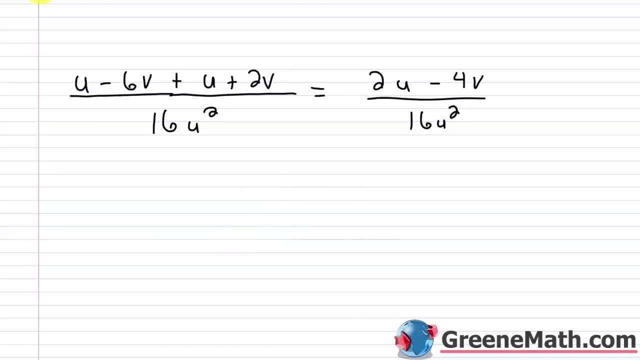 And all I really need to do is just factor it to see what the GCF would be. 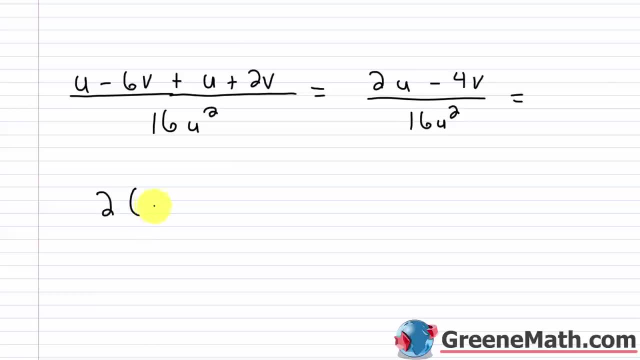 So in the numerator, I can pull out a 2. So this would be 2 times the quantity u minus 2v. In the denominator, I have a 16. 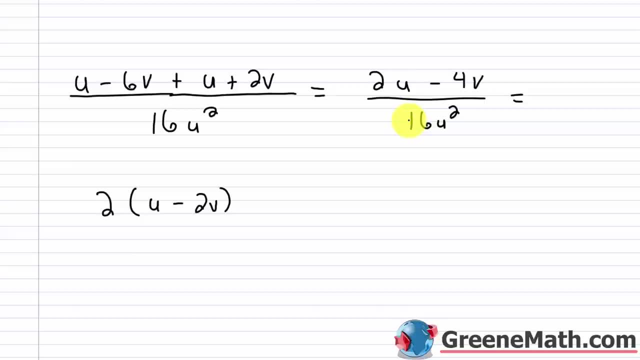 Now, I don't need to go through and write 2 times 2 times 2 times 2. I know 16 is 8 times 2. 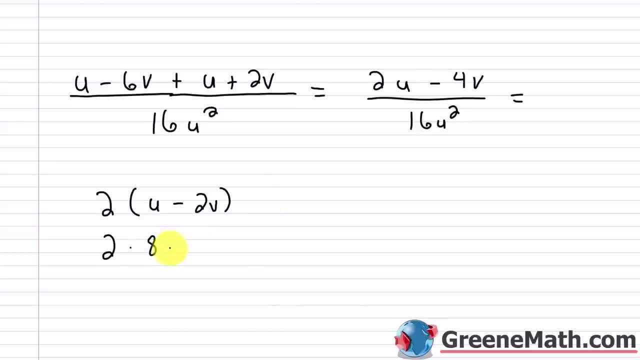 So I'll just write 2 times 8 and then times u squared. 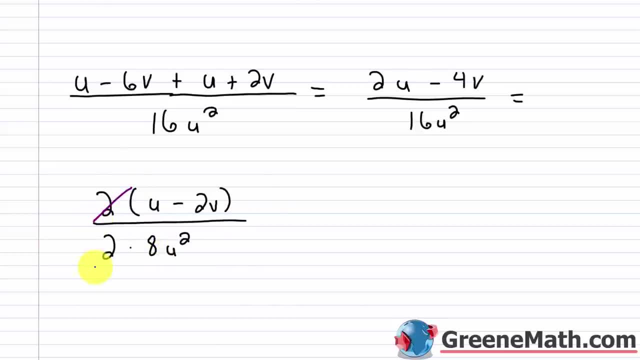 So I can see that I can cancel this factor of 2 with this factor of 2. 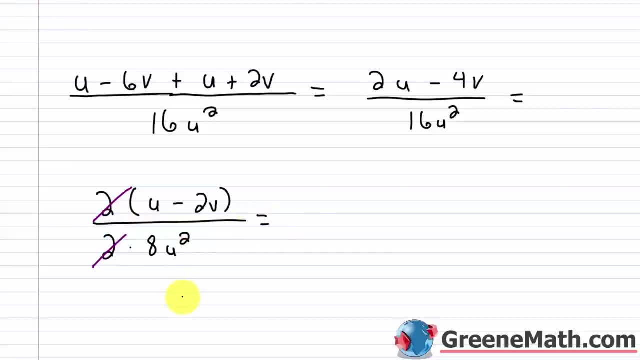 And so I have reduced this rational expression to its lowest terms. 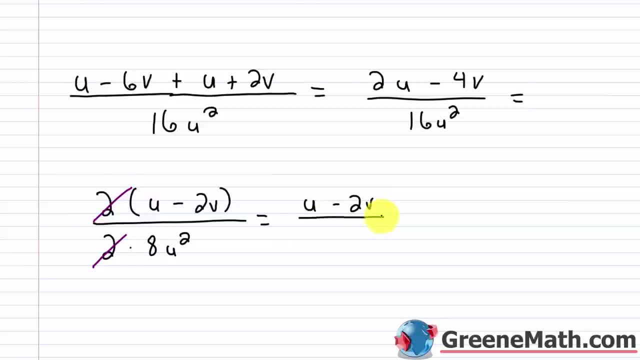 So I have u minus 2v as my simplified numerator over 8 u squared as my simplified denominator. And there's nothing else that I can do here. 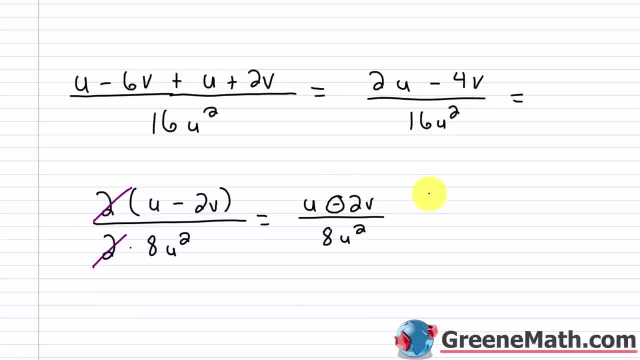 Remember, this is a subtraction sign. You can't go through and start going, 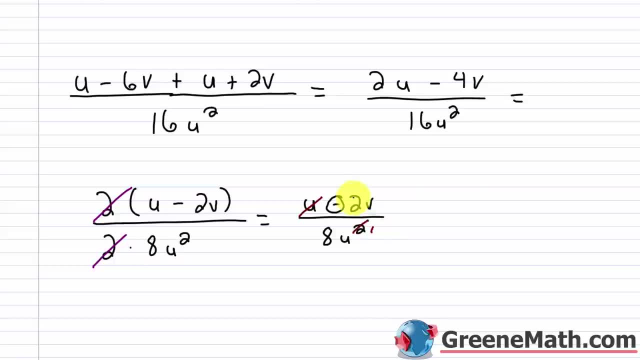 okay, this is going to cancel with this. I see that all the time. Or students will go, okay, this is going to cancel with this 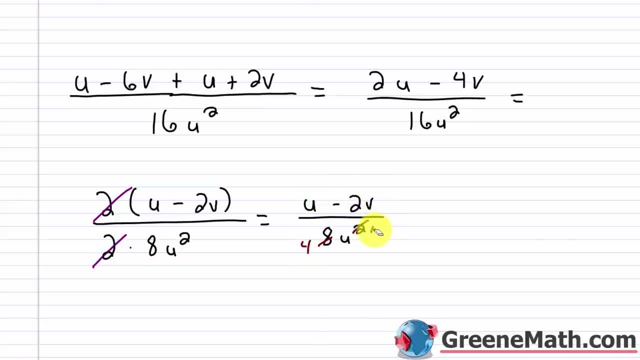 and that's going to give me a 4. That doesn't work that way. It's got to be factors. So we cancel common factors. 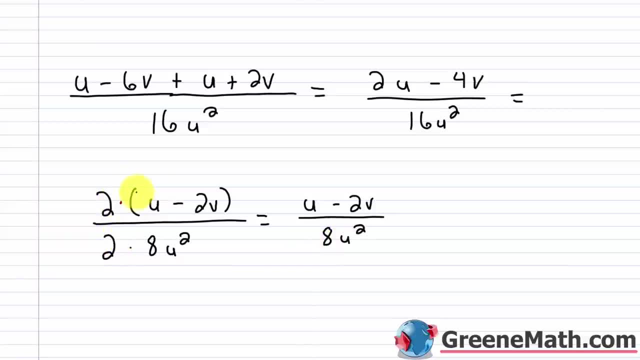 Here, this is multiplication. I am multiplying 2 by this u minus 2v, by that quantity. 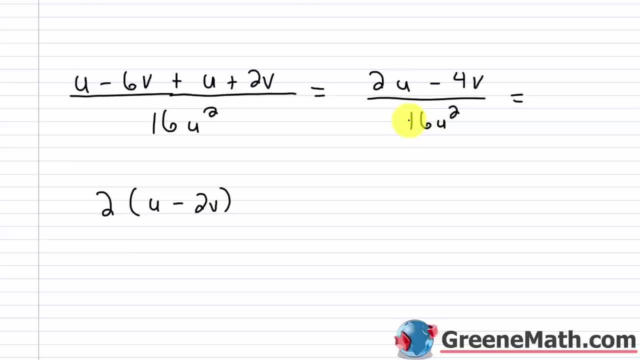 In the denominator, I have a 16.. Now I don't need to go through and write 2 times 2 times 2 times 2.. I know 16 is 8 times 2.. So I'll just write 2 times 8 and then times u squared. 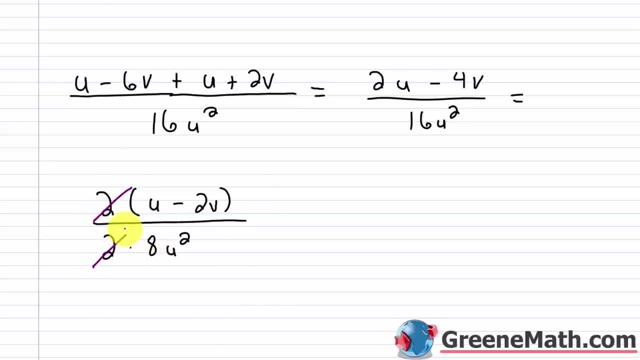 So I can see that I can cancel this factor of 2 with this factor of 2.. And so I have reduced this rational expression to its lowest terms. So I have u minus 2v as my simplified numerator, over 8, u squared as my simplified denominator. 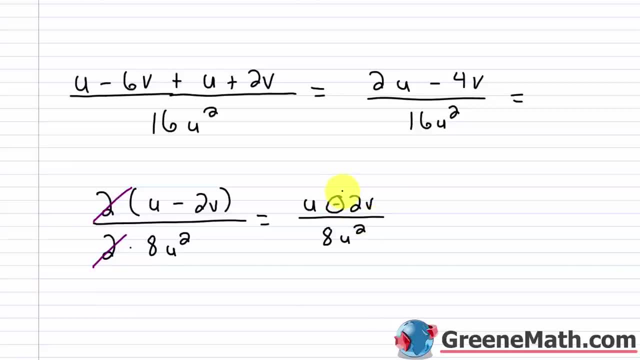 And there's nothing else that I can do here. Remember: this is a subtraction sign. You can't go through and start going: OK, this is going to cancel. with this, I see that all the time Or students will go: OK, well, this is going to cancel. 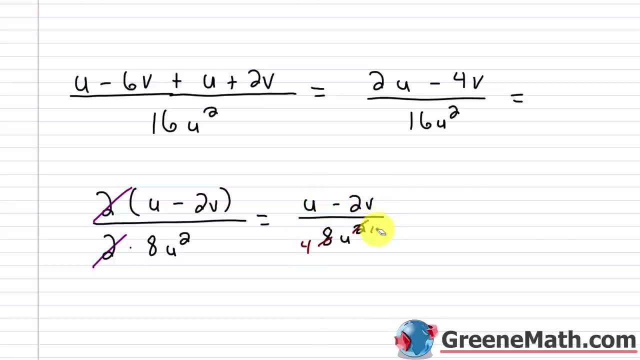 with this and that's going to give me a 4.. That doesn't work that way. It's got to be factors, right. So we cancel common factors Here. this is multiplication. I am multiplying 2 by this u minus 2v by that quantity. 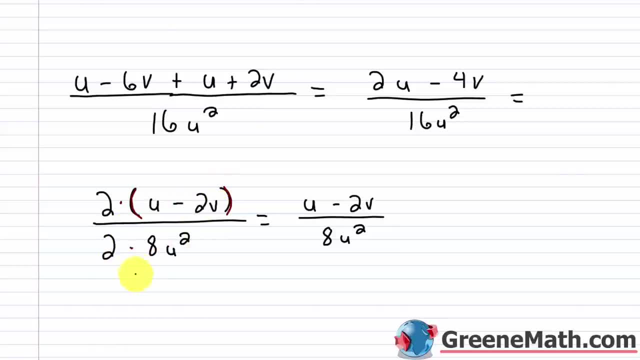 I am multiplying 2 by 8, u squared, So this is multiplication. These are factors. So I can cancel common factors When I think about u minus 2v. I can cancel common factors When I think about u minus 2v. these aren't factors, OK. 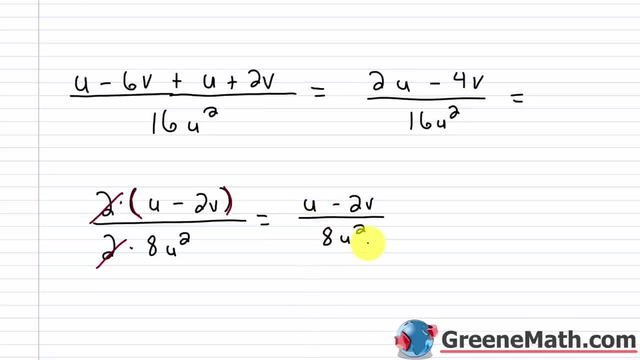 So I can't go through and just start canceling things. So it's very important that you understand that We cancel common factors, All right. so again, the answer here is: u minus 2v over 8, u squared. All right, let's take a look at another one. 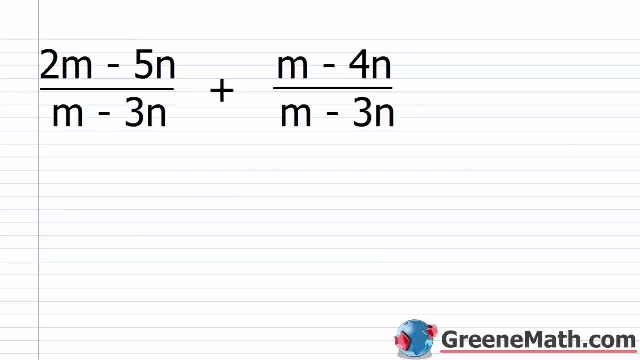 We have 2m minus 5n over m minus 3n, And then we're adding to this m minus 4n over m minus 3n. So again we have one with a common denominator of m minus 3n. 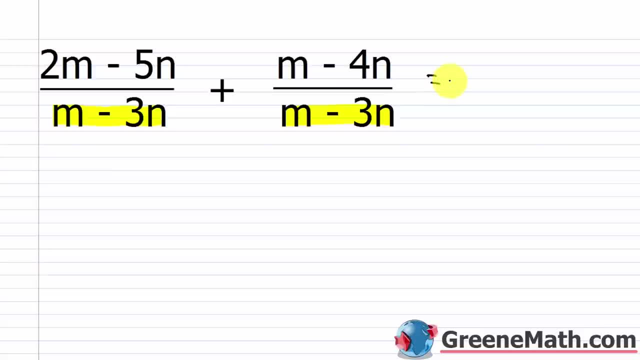 We're just going to leave that as it is And we're going to add the numerators. So the numerators: we have 2m minus 5n plus m minus 4n, over again that common denominator of m minus 3n. 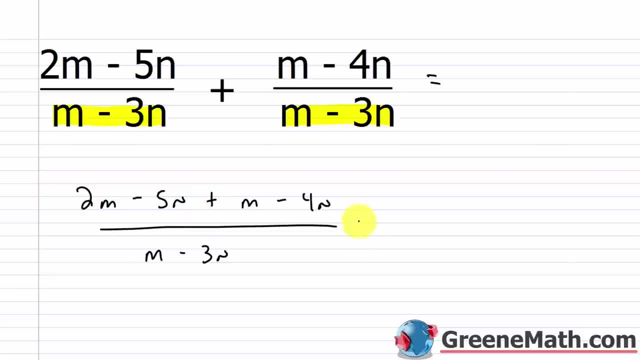 So just combine like terms here. So 2m plus m is 3m, This is 3m, And then negative 5n minus 4n is negative 9n, And this is over m minus 3n. So again I want to think about what. 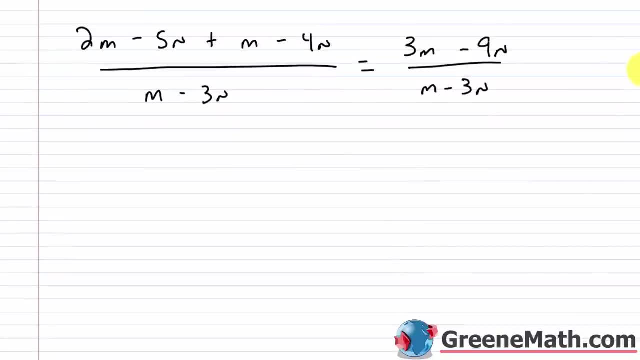 I can cancel. In some cases you're not going to be able to cancel anything. In other cases you're going to be able to cancel a lot. So if I look at m minus 3n, I can't factor that at all. 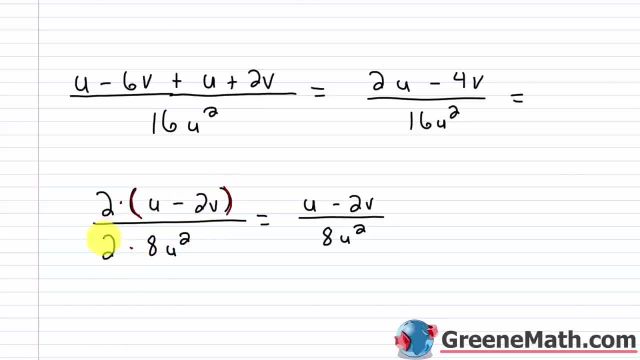 I am multiplying 2 by 8 u squared. So this is multiplication. 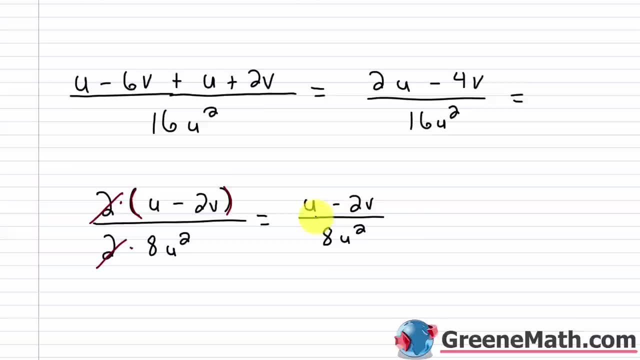 These are factors. So I can cancel common factors. 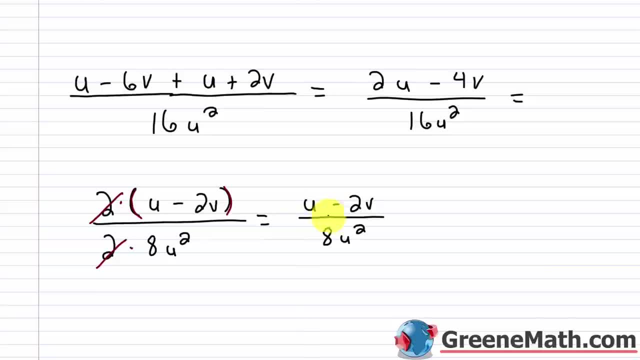 When I think about u minus 2v, these aren't factors. 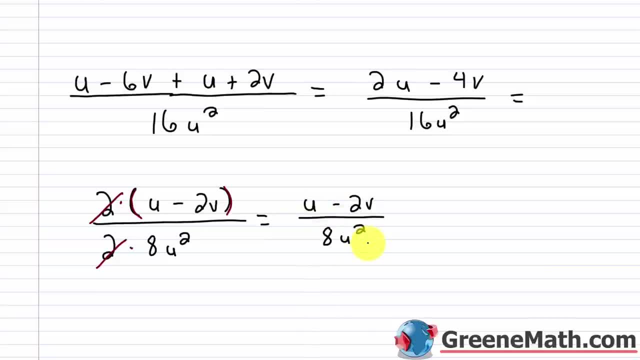 So I can't go through and just start canceling things. So it's very important that you understand that. 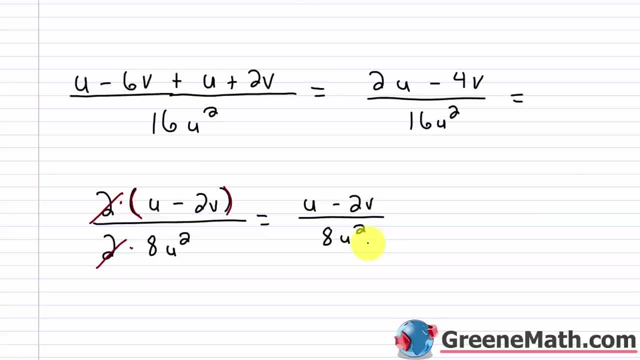 So again, the answer here is u minus 2v over 8 u squared. 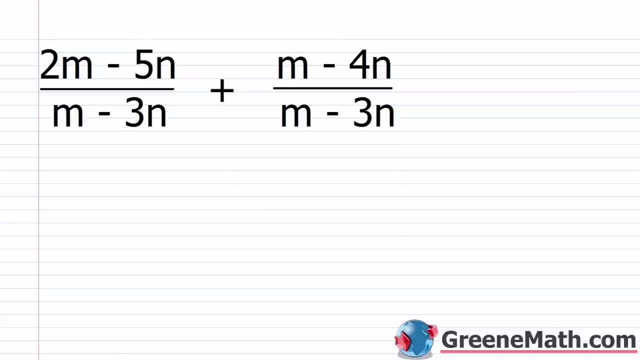 Let's take a look at another one. We have 2m minus 5n over m minus 3n. 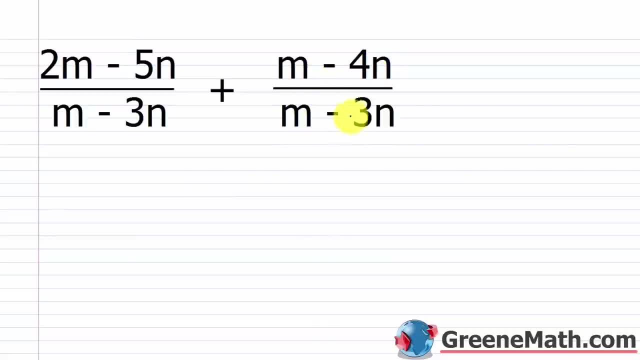 And then we're adding to this m minus 4n over m minus 3n. 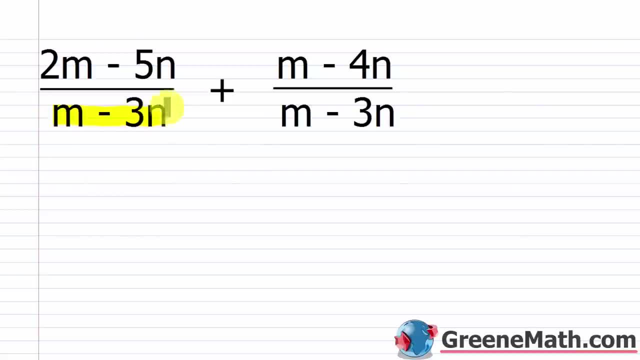 So again, we have one with a common denominator of m minus 3n. We're just going to leave that as it is. And we're going to add the numerators. So the numerators, we have 2m minus 5n plus m minus 4n over, again, that common denominator of m minus 3n. 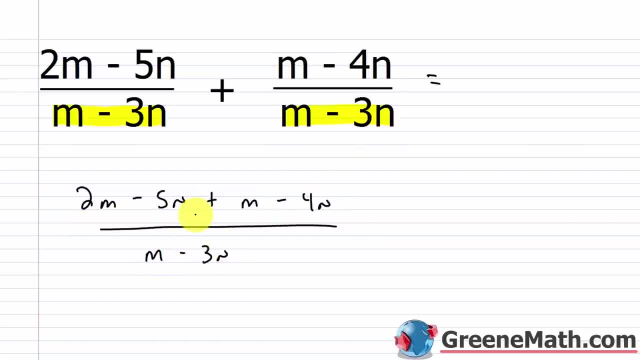 So just combine like terms here. So 2m plus m is 3m. This is 3m. 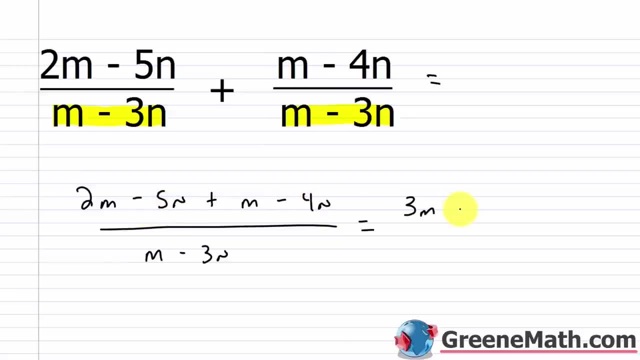 And then negative 5n minus 4n is negative 9n. 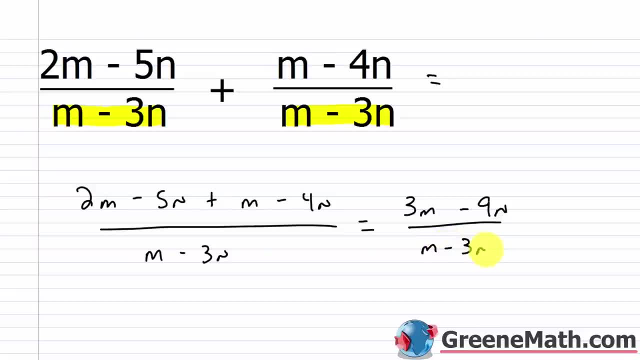 And this is over m minus 3n. 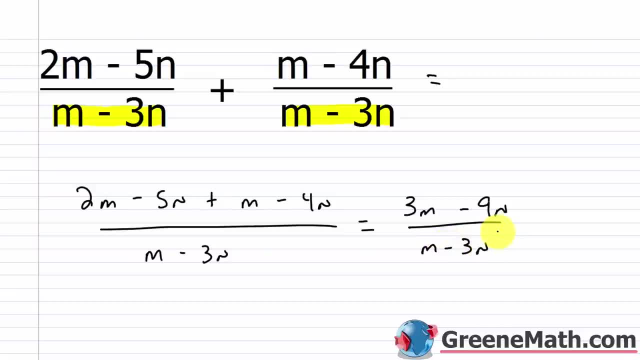 So again, I want to think about what I can cancel. 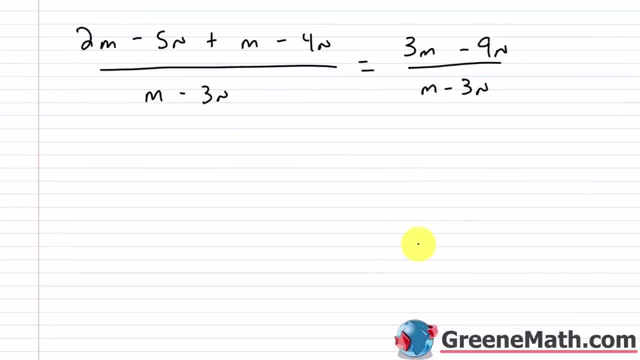 In some cases, you're not going to be able to cancel anything. In other cases, you're going to be able to cancel a lot. 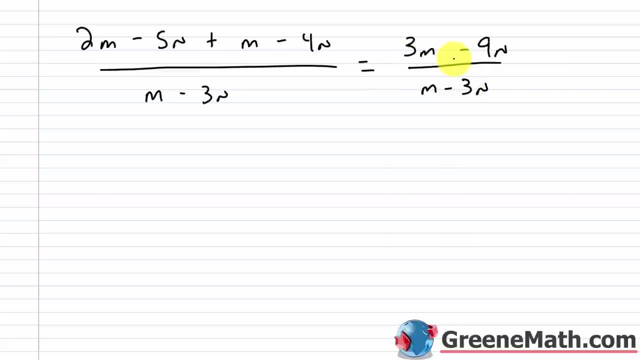 So if I look at m minus 3n, I can't factor that at all. If I look at 3m minus 9n, I can pull a 3 out. So let's just do that. Just pull out what you can and see what you get. So I'm going to pull out a 3. 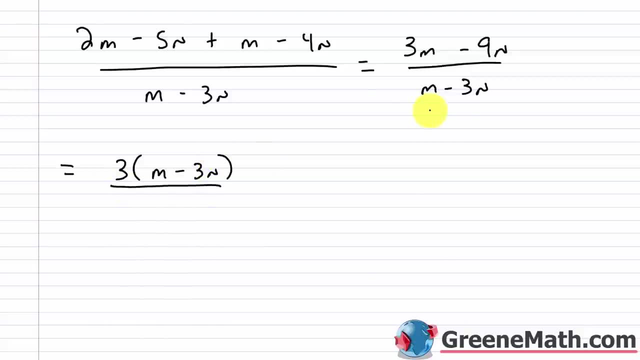 And I'll get m minus 3n inside. And we can see that now we have a common factor between numerator and denominator of m minus 3n. 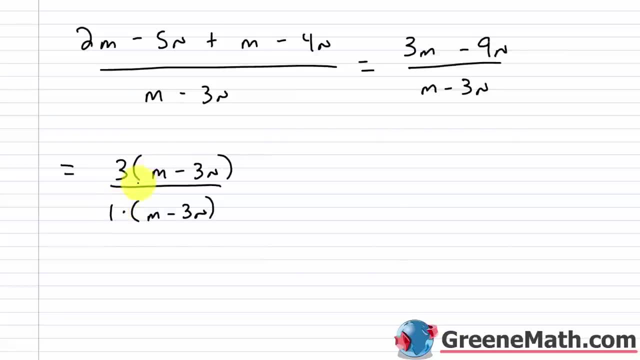 Again, if you want to, you can write this as times 1. So that's completely clear. 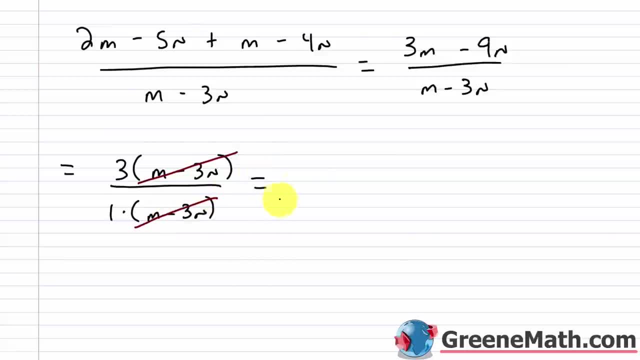 And then cancel this with this. And what I'm left with is 3 over 1, or just 3, as my simplified answer. 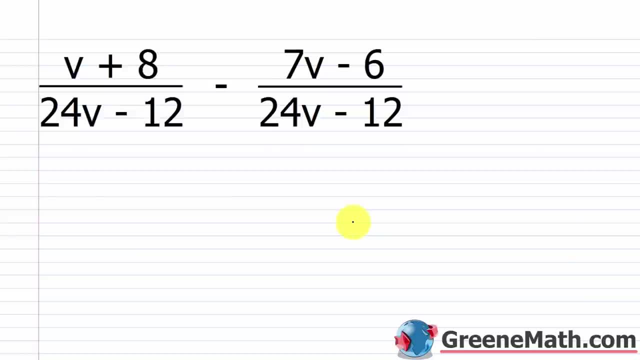 Okay, so now let's take a look at one with subtraction. 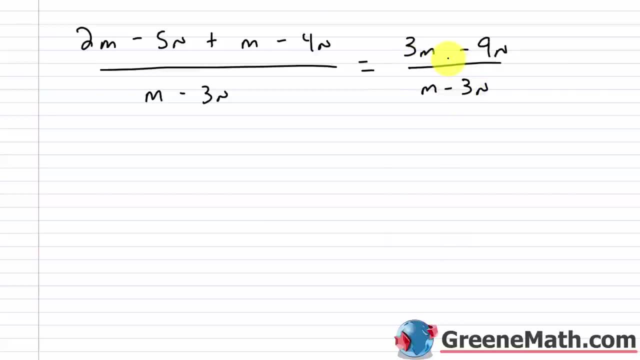 If I look at 3m minus 9n, I can pull a 3 out. So let's just do that. Just pull out what you can and see what you get. So I'm going to pull out a 3. And I'll get m minus 3n inside. 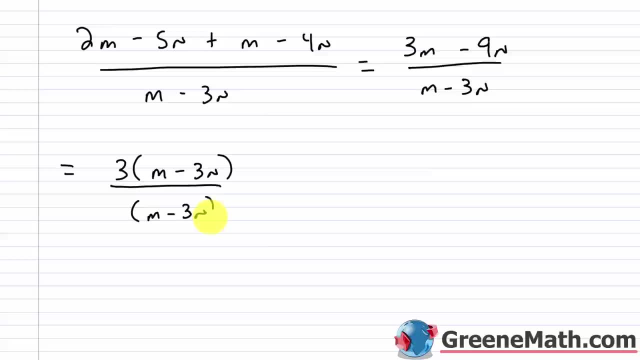 And we can see that now we have a common factor between numerator and denominator of m minus 3n. Again, if you want to, you can write: This is times 1.. So that's completely clear, And then cancel this with this. 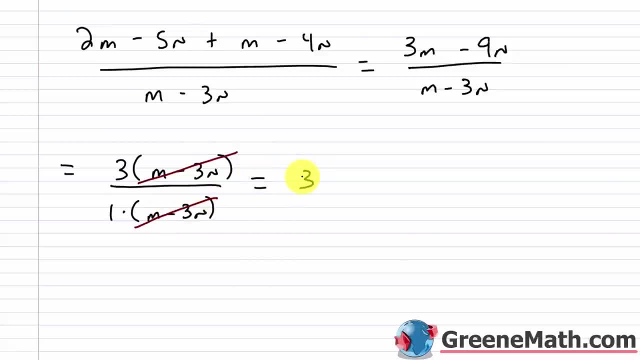 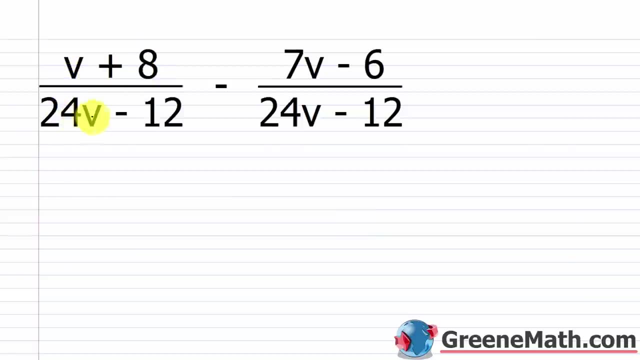 And what I'm left with is 3 over 1, or just 3, as my simplified answer. Okay, so now let's take a look at 1 with subtraction. So we have v plus 8 over 24v minus 12.. 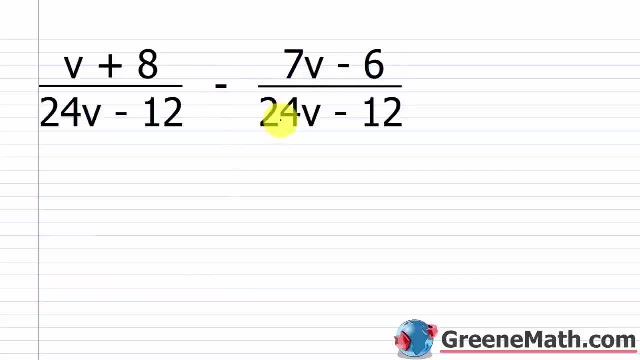 And I'm subtracting away 7v minus 6 over 24v minus 12.. Very important that you realize that this whole thing is being subtracted away. So that means I want to put my numerator Inside of parentheses when I go to do the subtracting. 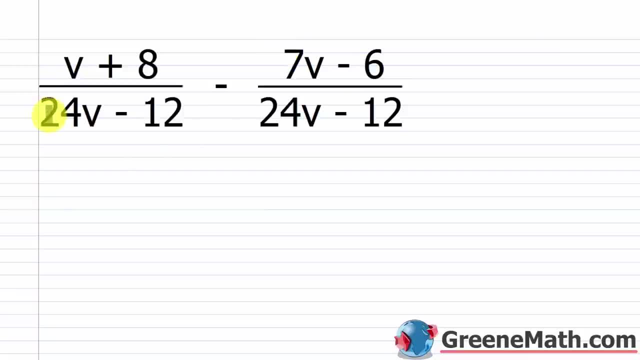 And we'll do that in a second. Now I have a common denominator. That common denominator is 24v minus 12.. So I'm just going to put 24v minus 12 down here And this is over. I have v plus 8 minus. 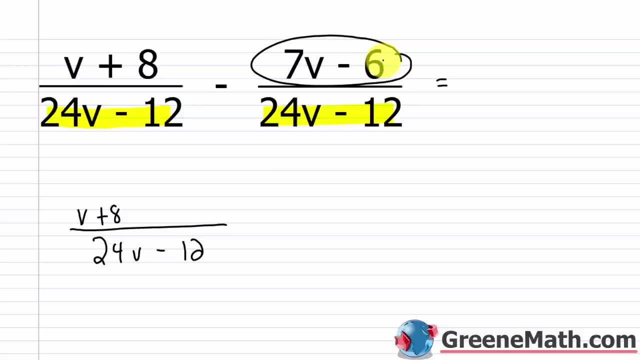 I'm subtracting this whole thing away. Please don't make the mistake of just putting minus 7v, minus 6. That is wrong. I am subtracting away the 7v And the negative 6.. So there's kind of two things you can do. 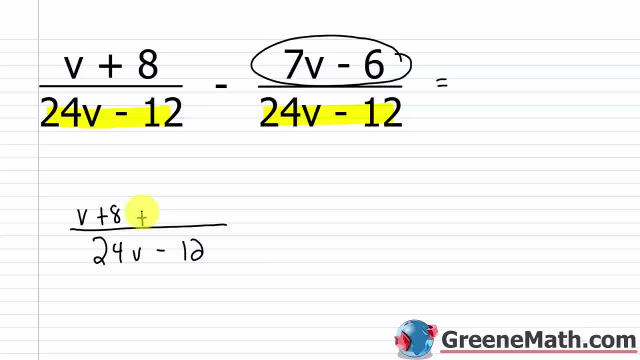 You can change this to plus. Okay, this to plus, And then you can change the sign of each term. So this could be plus negative 7v, And then, since this is negative 6,, it would be positive 6.. You can do that. 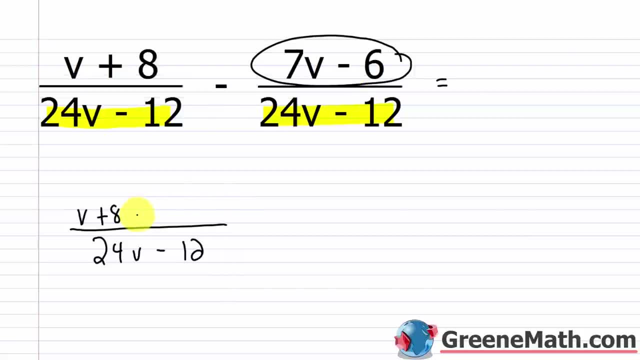 Or you can do it kind of the slower way And just put a minus sign out in front of parentheses, So 7v minus 6.. But again, if you see a negative outside of some parentheses, what do you do In order to drop the parentheses? 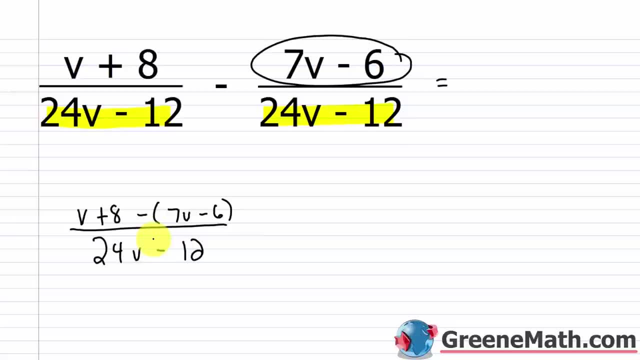 You've got to change the sign of each term inside. Remember, multiplying by that phantom, negative 1.. So we can do plus negative 1.. Again, negative 1 times 7v is negative 7v, And then negative 1 times negative 6 is plus 6.. 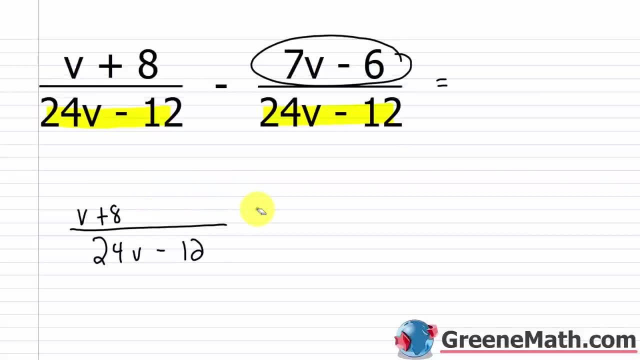 So, any kind of way that you look at it, it's going to be minus 7v, minus 7v and plus 6.. Okay, so if we combine like terms, v minus 7v is negative 6v, And then 8 plus 6 is 14.. 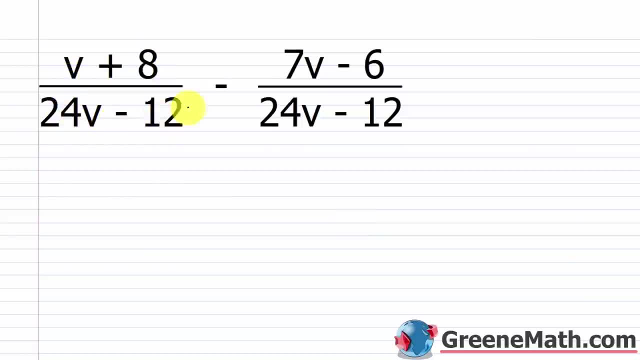 So we have v plus 8 over 24v minus 12. And I'm subtracting away 7v minus 6 over 24v minus 12. 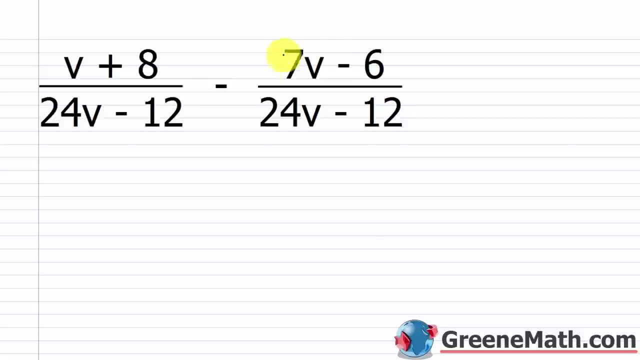 Very important that you realize that this whole thing is being subtracted away. 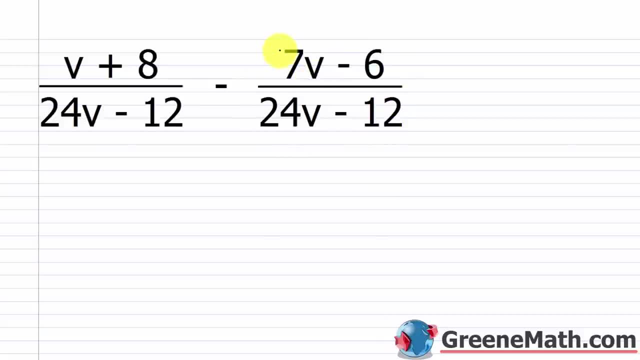 So that means I want to put my numerator inside of parentheses when I go to do the subtracting. We'll do that in a second. 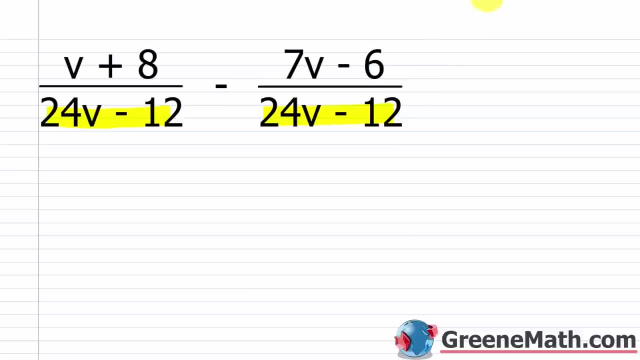 That common denominator is 24v minus 12. So I'm just going to put 24v minus 12 down here. And this is over. 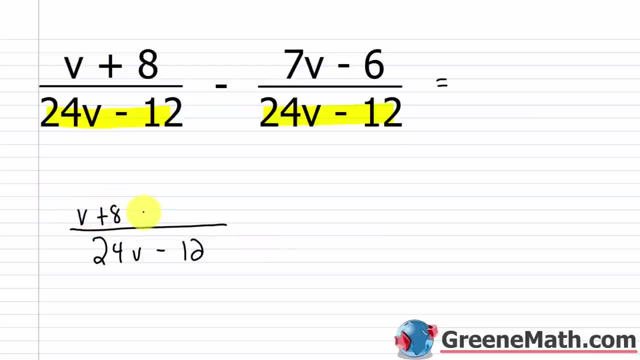 I have v plus 8 minus I'm subtracting this whole thing away. 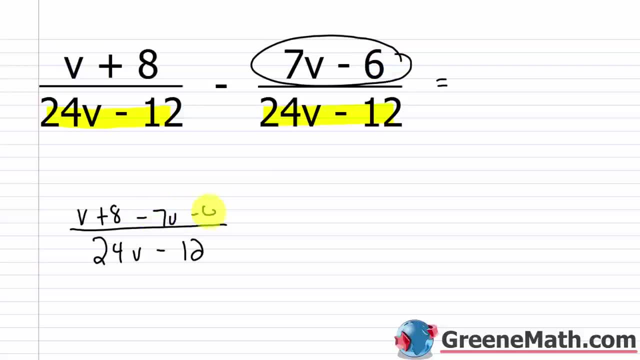 Please don't make the mistake of just putting minus 7v minus 6. That is wrong. 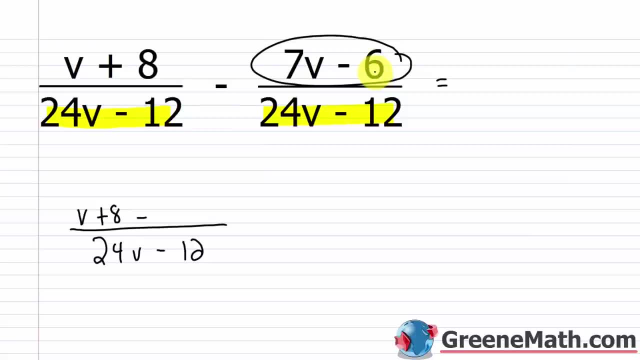 I am subtracting away the 7v and the negative 6. So there's kind of two things you can do. 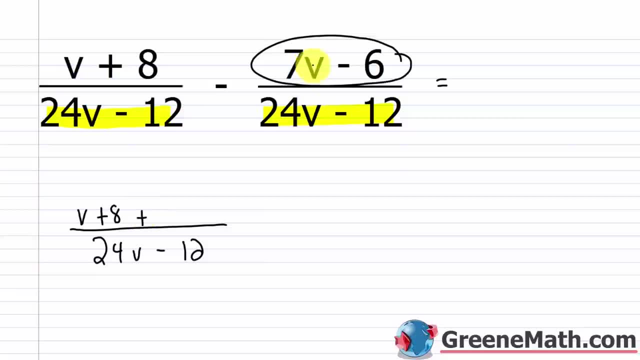 You can change this to plus. And then you can change the sign of each term. So this could be plus negative 7v. 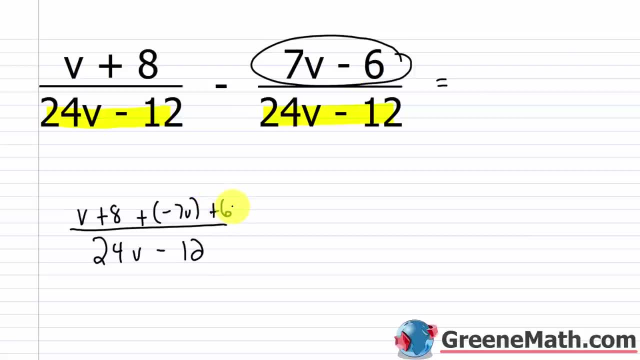 And then since this is negative 6 it would be positive 6. You can do that. 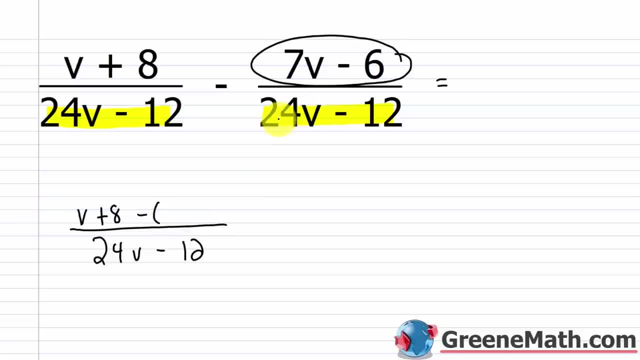 Or you can do it kind of the slower way. You just put a minus sign out in front of parentheses. 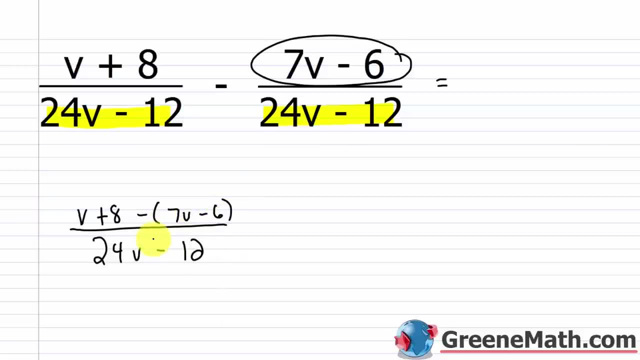 So 7v minus 6. But again if you see a negative outside of some parentheses what do you do? In order to drop the parentheses you've got to change the sign of each term inside. Remember multiplying by that phantom negative 1. So we can do plus negative 1. Again negative 1 times 7v is negative 7v. And then negative 1 times negative 6 is plus 6. 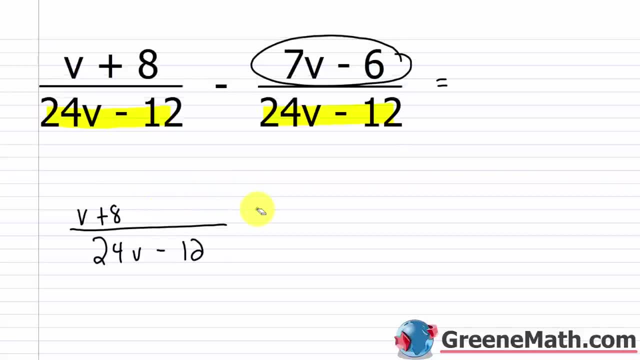 So any kind of way that you look at it it's going to be minus 7v minus 7v and plus 6. So if we combine like terms v minus 7v is negative 6v and then 8 plus 6 is 14. So plus 14 this is over 24v minus 12. 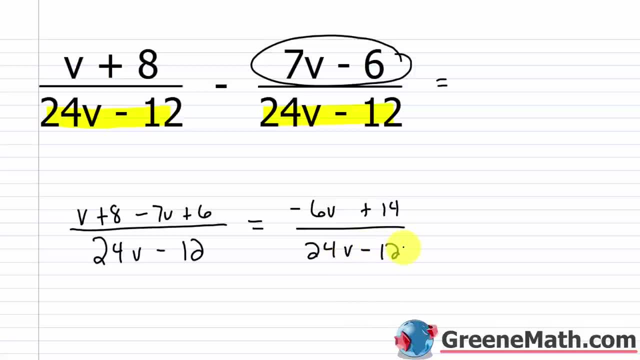 Now again we want to look to see if we can simplify anything before we report our answer. 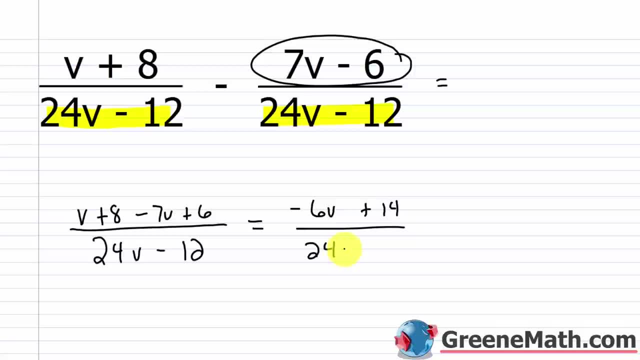 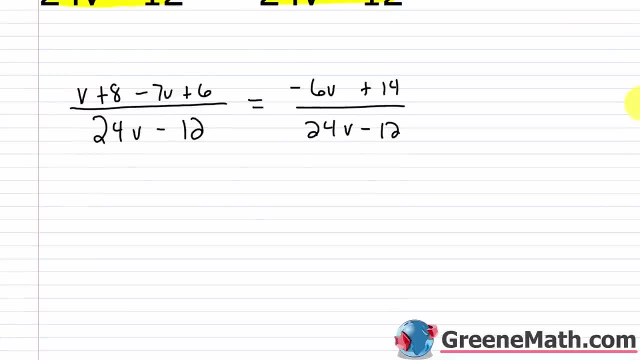 So plus 14.. This is over 24v minus 12.. Now again we want to look to see if we can simplify anything before we report our answer. I know in the numerator I can pull out a 2.. I could also pull out a negative 2 if I wanted to, which is just kind of up to me. 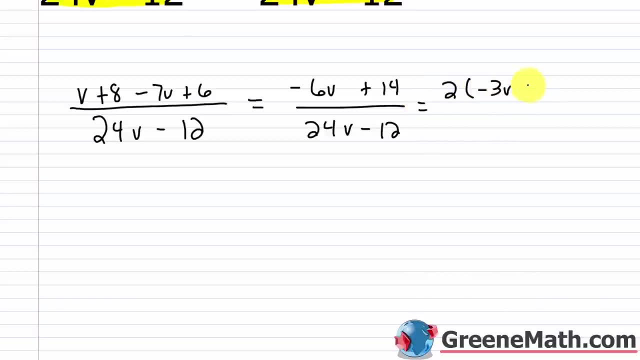 Let's just pull out a 2. And I'd have negative 3v plus 7.. Down here, let's also pull out a 2. And I'll have 12v minus 6.. Now I can't really factor this any further. 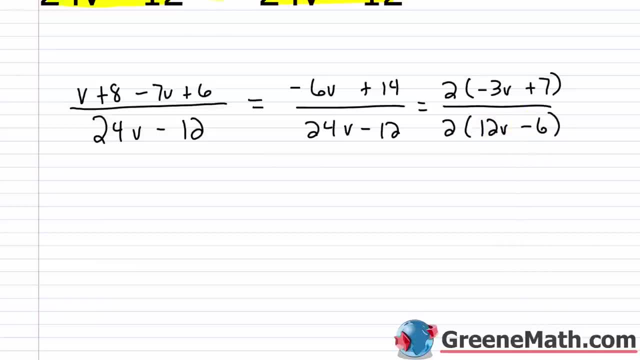 So I really don't need to do anything else Down here. I would just cancel this common factor of 2 between numerator and denominator And then I will report my answer as negative: 3v plus 7 over 12v minus 6.. 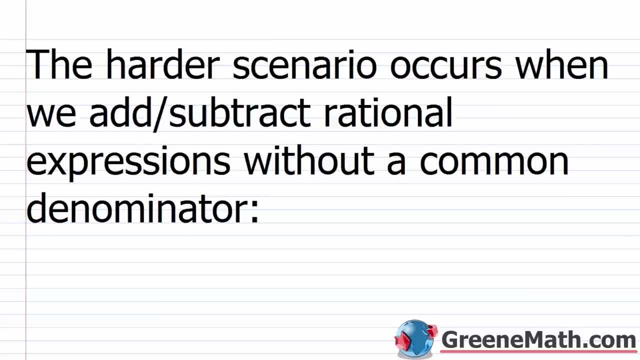 All right. so the harder scenario occurs when we add or subtract rational expressions without a common denominator. It's the same thing as if we added or subtracted fractions without a common denominator. You've got all these extra steps. So with fractions, if I have something like, let's say, 1 fourth plus, 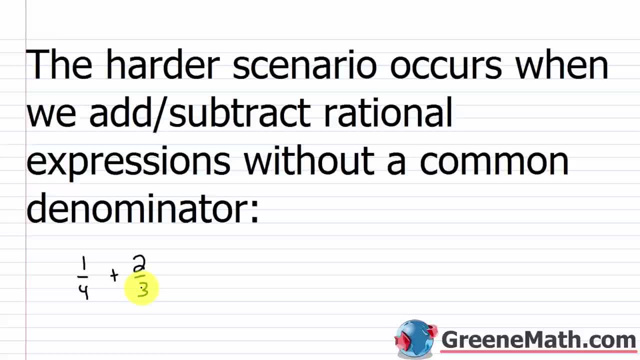 2 thirds. I find my LCD. In this particular case, the LCD is 4 times 3, or 12.. I change each fraction into an equivalent fraction, where 12 is the denominator. So I multiply this by 3 over 3.. 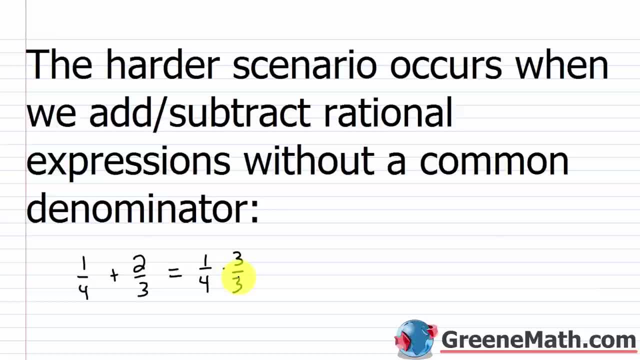 Remember that's a complicated form of 1. So it just changes the way it looks, not the value. So it's still worth 1 fourth in the end. Then plus, I'll have 2 thirds. I'm going to multiply this by 4 over 4.. 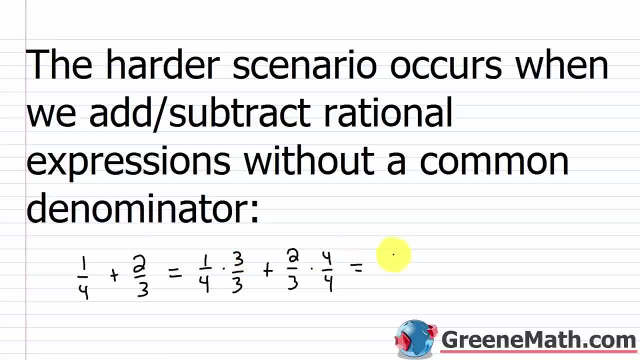 Again just a common denominator. So I multiply this by 4 over 4.. I get a complicated form of 1. So 1 times 3 is 3.. Over 4 times 3 is 12.. Then plus 2 times 4 is 8.. 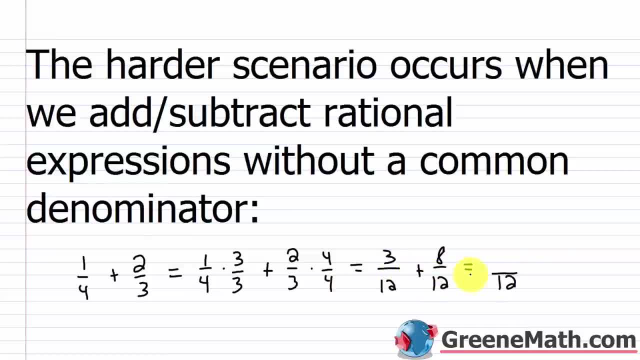 Over 3 times 4 is 12.. Then we have a common denominator. So we just put the common denominator there, We add the numerators: 3 plus 8 is 11. So I get 11 twelfths there. 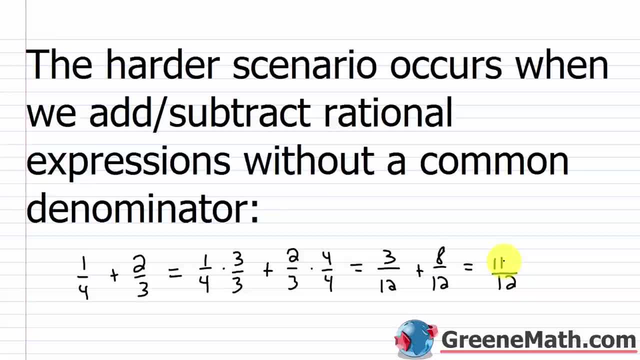 So it's the same process for adding and subtracting rational expressions without a common denominator. It's just the fact that you have variables involved. It's very easy and very, very tedious, depending on what level problem you're looking at. All right. 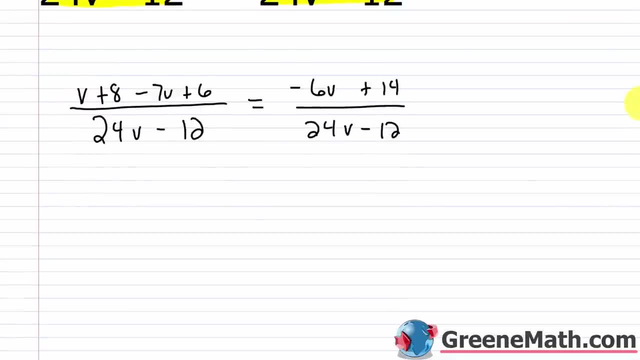 I know in the numerator I can pull out a 2. I could also pull out a negative 2 if I wanted to which is just kind of up to me. Let's just pull out a 2 and I'd have negative 3v plus 7. 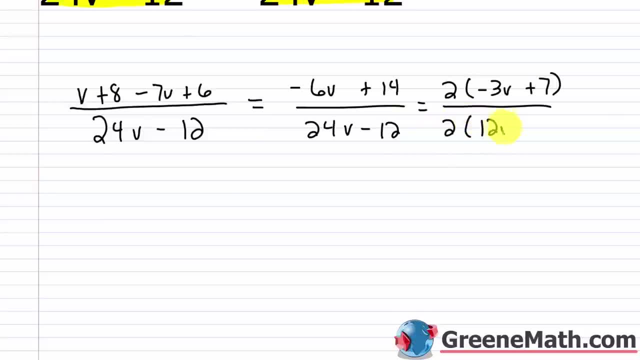 Down here let's also pull out a 2 and I'll have 12v minus 6. 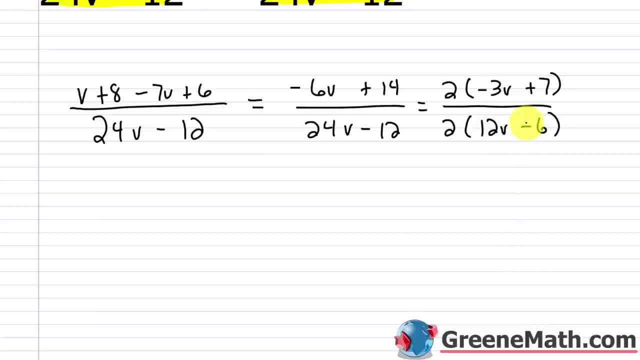 Now I can't really factor this any further so I really don't need to do anything else down here. I would just cancel this common factor of 2 between numerator and denominator. 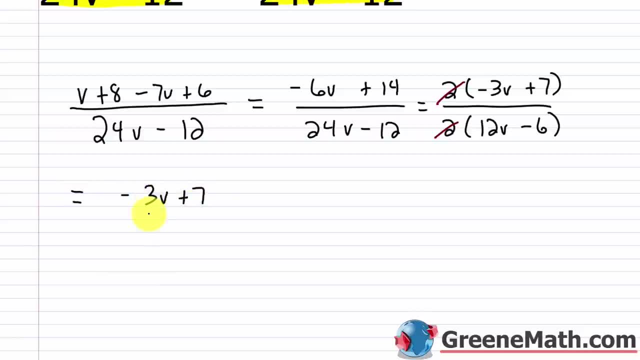 I will report my answer as negative 3v plus 7 over 12v minus 6. 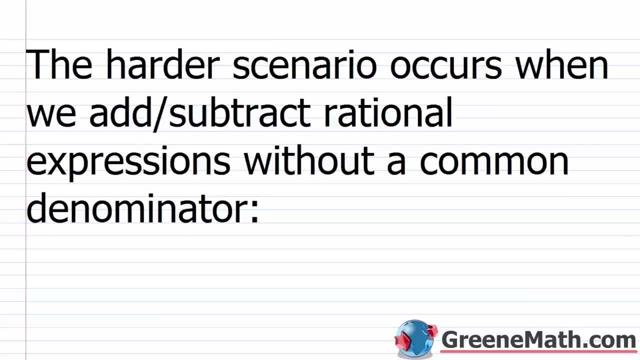 Alright so the harder scenario occurs when we add or subtract rational expressions without a common denominator. It's the same thing as if we added or subtracted fractions without a common denominator. You've got all these extra steps. 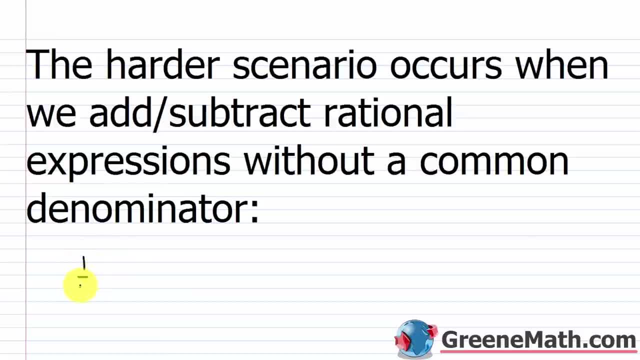 So with fractions if I have something like let's say 1 fourth plus 2 thirds I find my LCD in this particular case is 4 times 3 or 12. 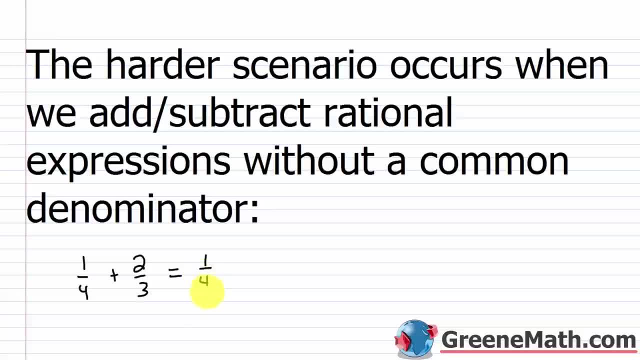 I change each fraction into an equivalent fraction where 12 is the denominator. So I multiply this by 3 over 3. Remember that's a complicated form of 1 so it just changes the way it looks not the value. So it's still worth 1 fourth in the end. 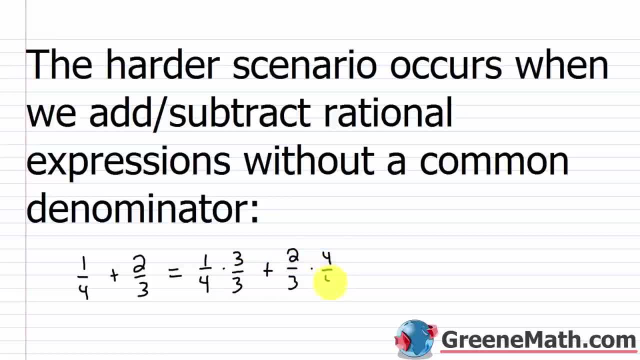 Then plus I'll have 2 thirds I'm going to multiply this by 4 over 4. Again just a complicated form of 1. So 1 times 3 is 3 over 4 times 3 is 12. Then plus 2 times 4 is 8 over 3 times 4 is 12. Then we have a common denominator so we just put the common denominator there and we add the numerators. 3 plus 8 is 11. 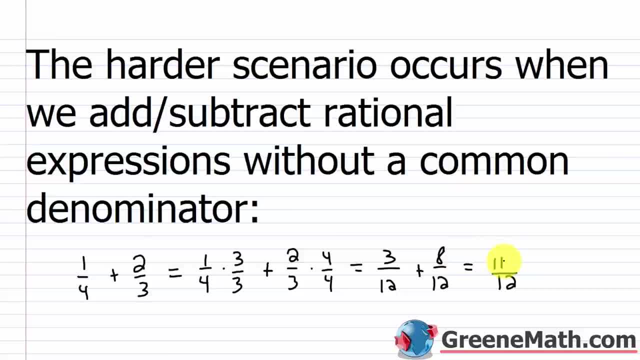 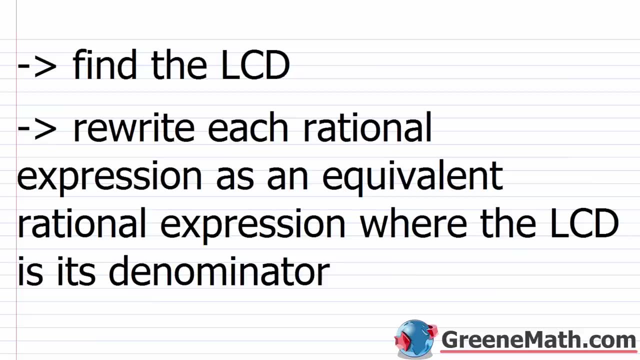 So I get 11 twelfths there. So it's the same process for adding and subtracting rational expressions without a common denominator. It's just the fact that you have variables involved you have to factor stuff. It just gets very very messy and very very tedious depending on what level problem you're looking at. 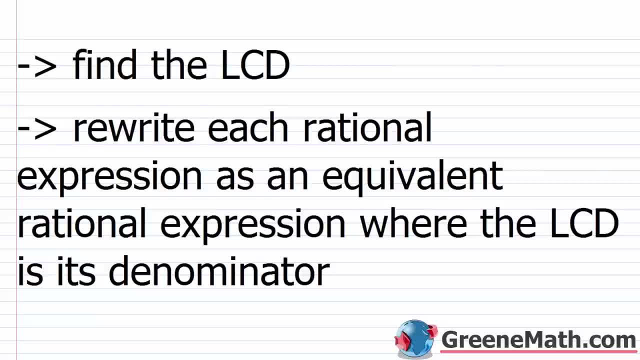 So the first thing we want to do is find the LCD Again, the least common denominator. We learned how to do that for a group of rational expressions in our last lesson. If you don't know how to do that at this point, if you start watching more of this video and 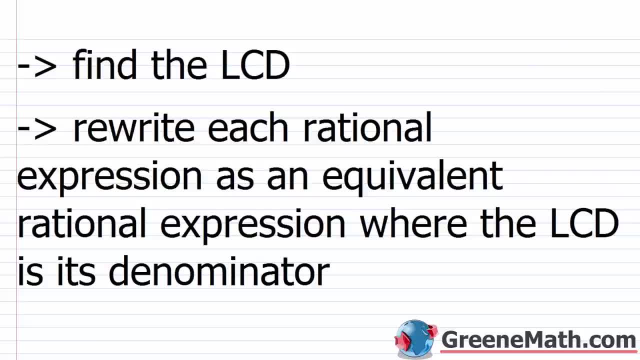 you get very, very confused. please stop, Go back to that video and watch that, Get fully up to speed on how to find the LCD and then come back. It's very, very difficult to do this if you've missed a step. 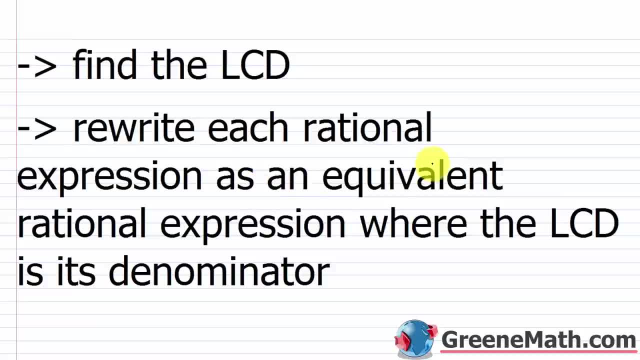 The next thing you're going to do is you're going to rewrite each rational expression as an equivalent rational expression where the LCD is its denominator, Just like we did with the fractions when we were adding them a minute ago. All right, Then we want to add or subtract numerators and then simplify. 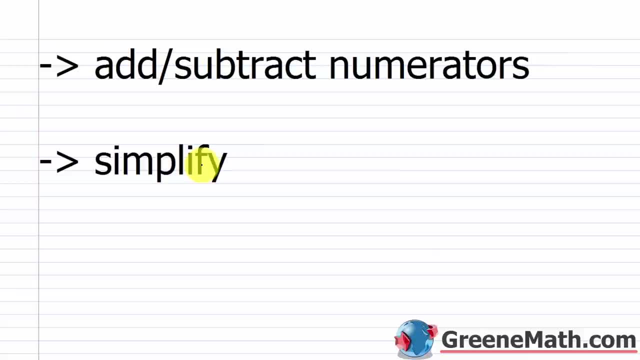 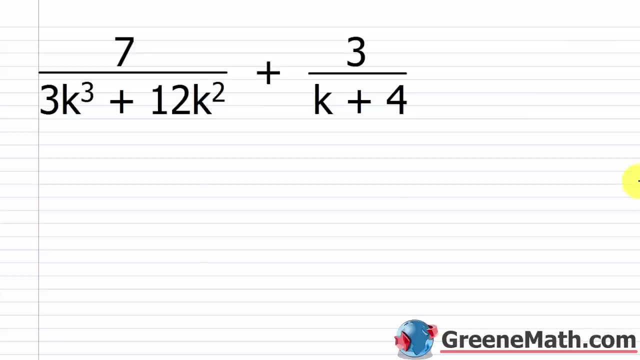 So very, very simple overall procedure-wise. Just again, if you're working with something that's very long and tedious, it just gets kind of irritating sometimes. So let's start out with this first one. We have 7 over 3k cubed plus 12k squared, plus 3 over k plus 4.. 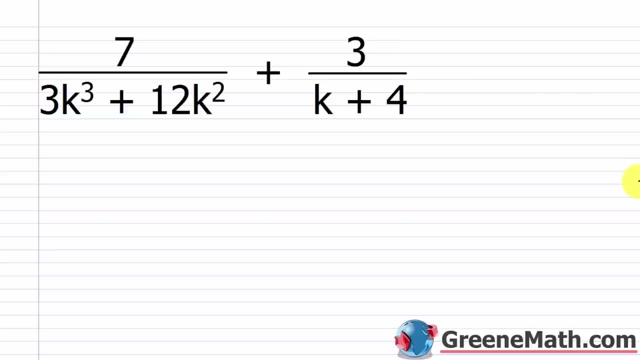 So the first thing I want to do is I want to find my LCD. So the way I do that is I factor each denominator. So if I factor this denominator, I could pull out a 3k squared, and that would leave me with what? 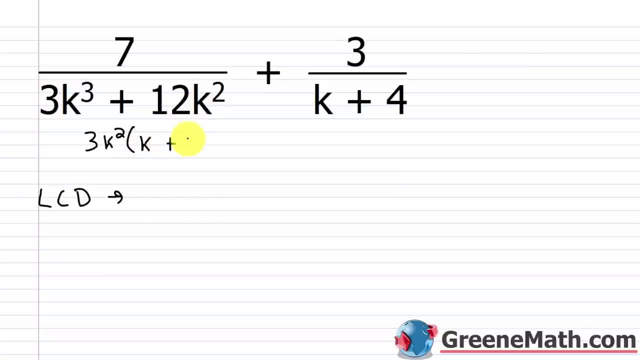 I pull that out from here, I'd get k And then plus. if I pull that out from here, I would have a 4. Now this over here is k plus 4.. So really, if I look at the LCD, it's going to be really simple. 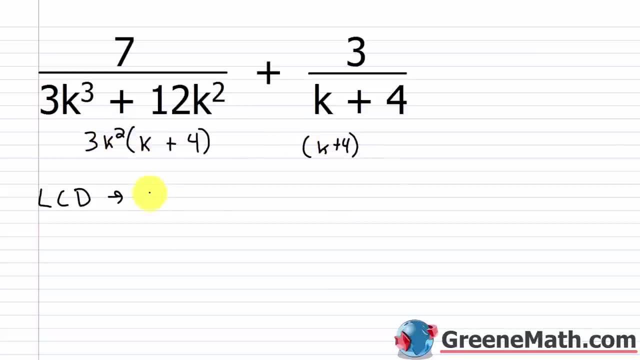 If I look at the LCD, it's going to be what It's going to be: 3k squared times k plus 4.. So 3k squared times k plus 4.. So this is okay. I don't need to make any changes to that rational expression. 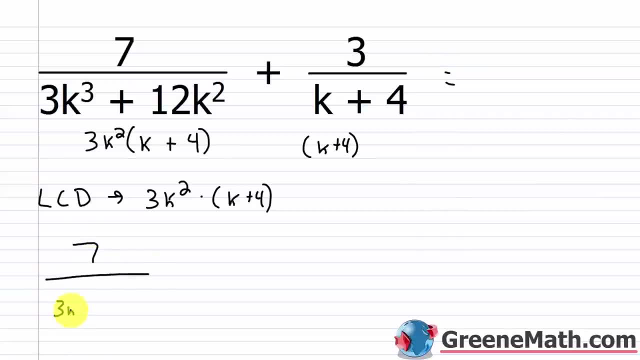 So I can leave it as it is: 7 over 3k squared times the quantity k plus 4.. Then plus For this guy over here, we have 3 over k plus 4.. Now what would I need to multiply k plus 4 by? to make the denominator the same. 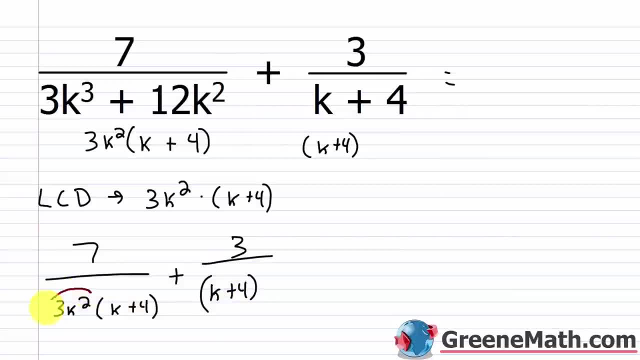 Well, this is what I'm missing: This factor of 3k squared. So I would multiply the denominator by 3k squared And to make that legal, I need to also multiply the numerator by 3k squared, Because I want to multiply by 1.. 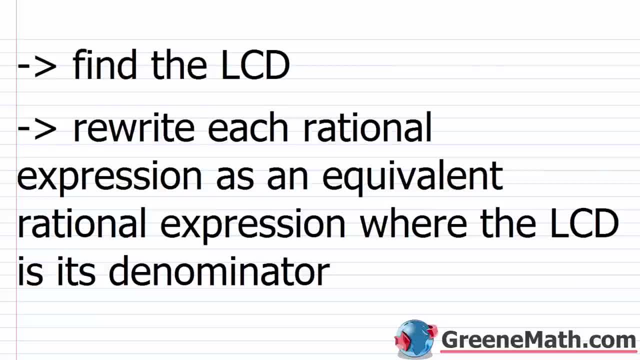 So the first thing we want to do is find the LCD again the least common denominator. We learned how to do that for a group of rational expressions in our last lesson. If you don't know how to do that at this point if you start watching more of this video and you get very very confused please stop, go back to that video and watch that get fully up to speed on how to find the LCD and then come back. 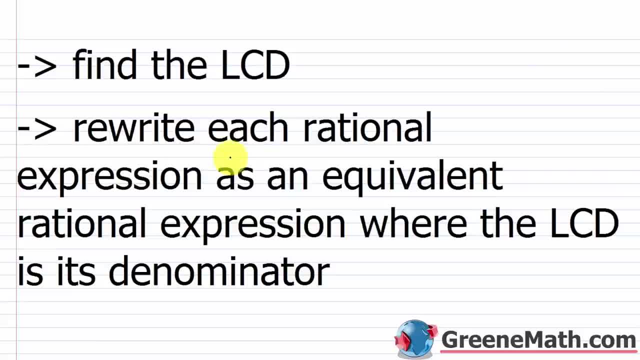 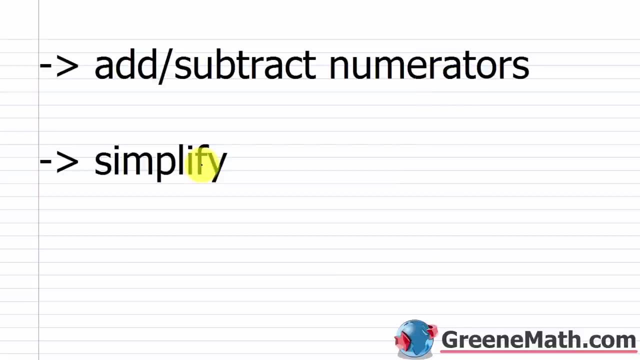 It's very very difficult to do this if you've missed a step. The next thing you're going to do is you're going to rewrite each rational expression where the LCD is its denominator. Just like we did with the fractions when we were adding them a minute ago. Then we want to add or subtract numerators and then simplify. 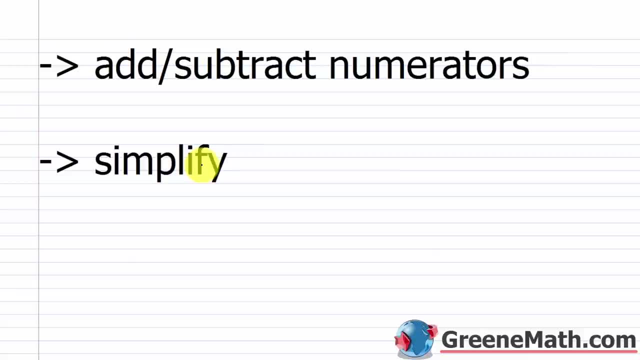 Very very simple overall procedure wise just again if you're working with something that's very long and tedious it just gets kind of irritating sometimes. 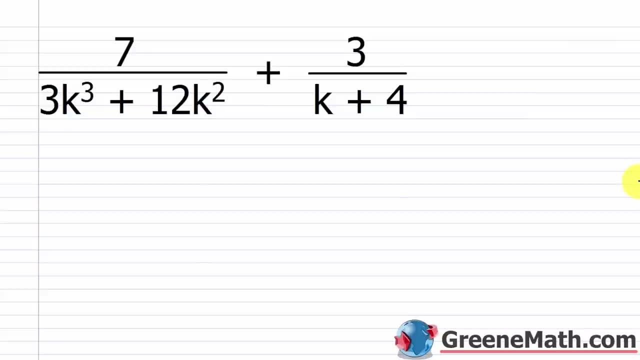 So let's start out with this first one. We have 7 over 3k cubed plus 12k squared plus 3 over k plus 4. So the first thing I want to do is I want to find my LCD. 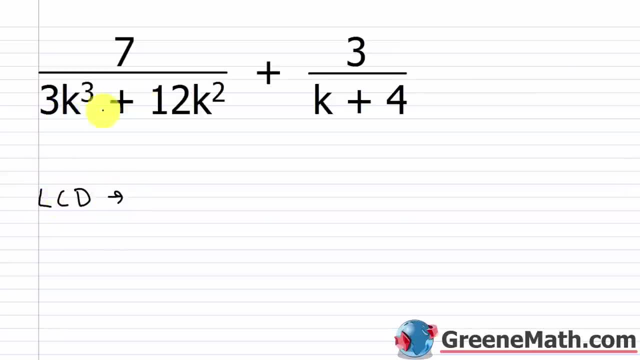 So the way I do that is I factor each denominator. So if I factor this denominator I could pull out a 3k squared and that would leave me with what? I pull that out from here I'd get k and then plus if I pull that out from here I would have a 4. Now this over here is k plus 4. 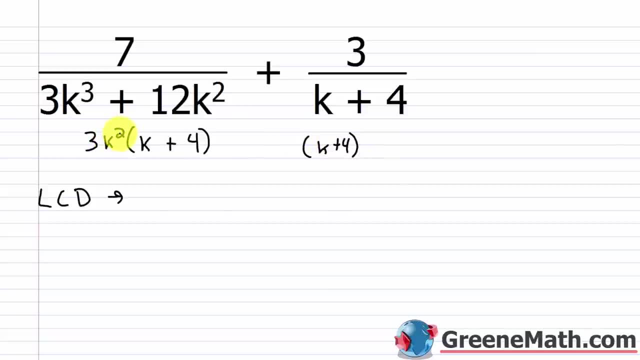 So really if I look at the LCD it's going to be what? 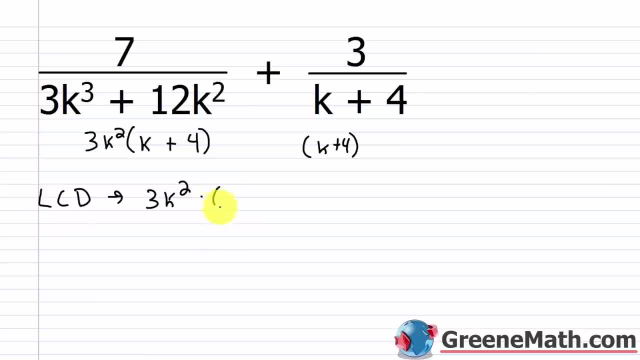 It's going to be 3k squared times k plus 4. So 3k squared times k plus 4. So this is going to be I don't need to make any changes to that rational expression. 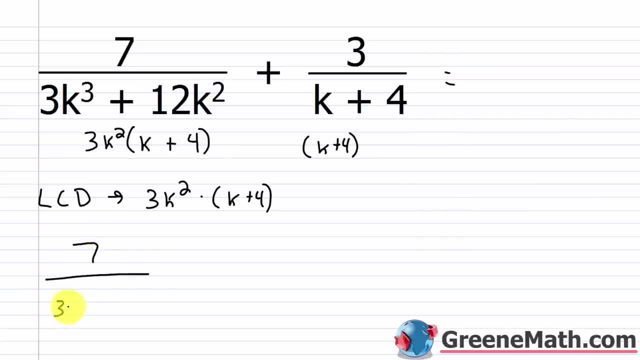 So I can leave it as it is 7 over 3k squared times the quantity k plus 4 then plus for this guy over here we have 3 over k plus 4. 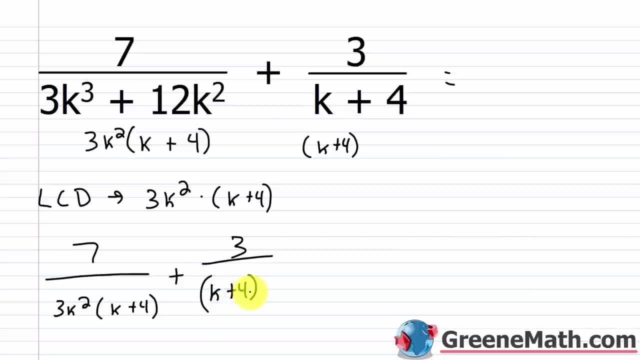 Now what would I need to multiply k plus 4 by to make the denominator the same as this? 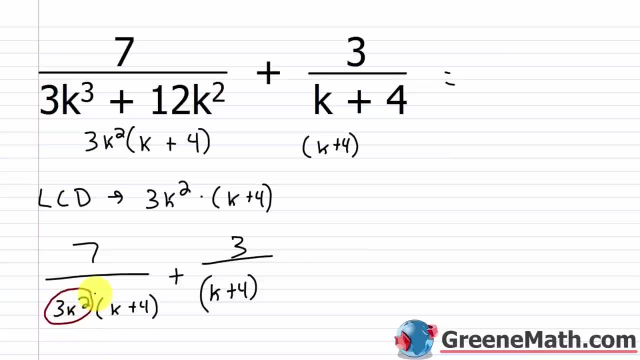 Well this is what I'm missing this factor of 3k squared. 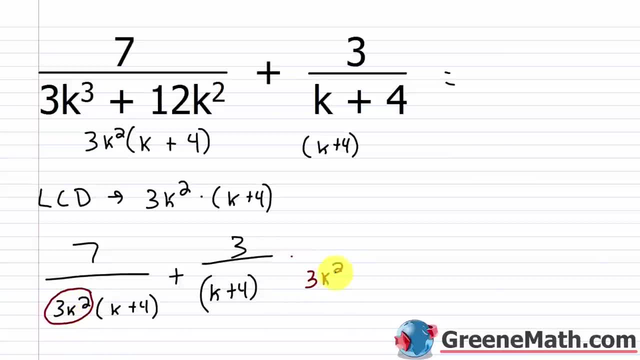 So I would multiply the denominator by 3k squared 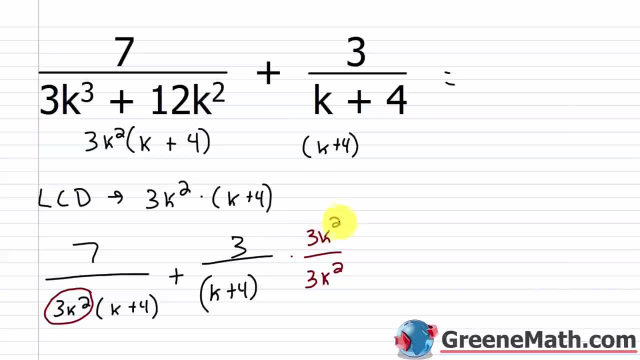 and if that's not legal I need to also multiply the numerator by 3k squared because I want to multiply by 1. 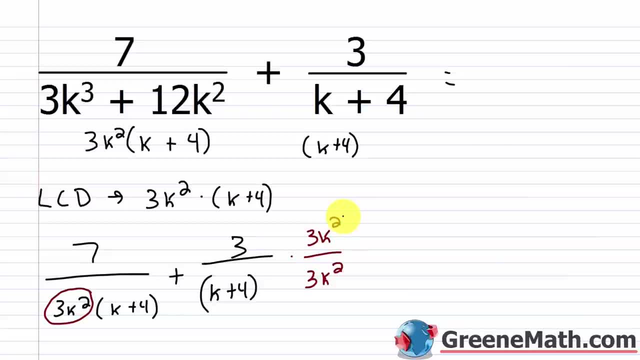 3k squared over 3k squared is 1. Just a complicated form of 1 but it's still 1. Now if I multiply here 3 times 3k squared is 9k squared. Let's scroll down a little bit. 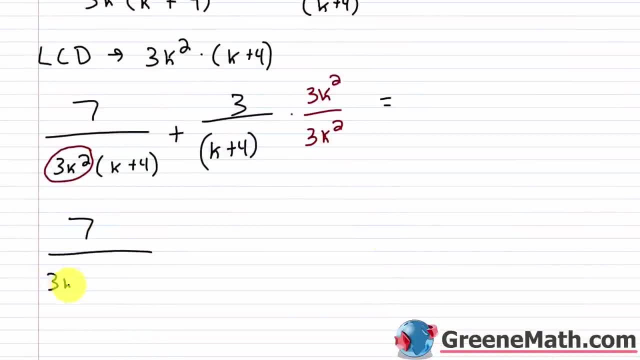 So this equals I'll rewrite this first 7 over again 3k squared times the quantity k plus 4 3 times 3k squared is 9k squared and this is over 3k squared times the quantity k plus 4. So 3k squared times the quantity k plus 4 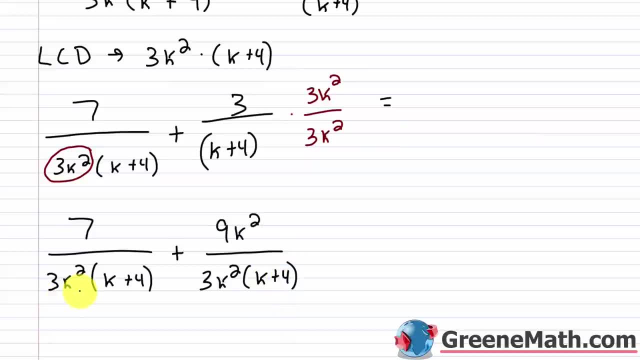 So now I have a common denominator. This denominator is the same as this denominator so I can just add the numerators and so basically what I'd have is just 9k squared plus 7 over that common denominator of 3k squared times the quantity k plus 4 and in this particular case there's nothing I can do to simplify. 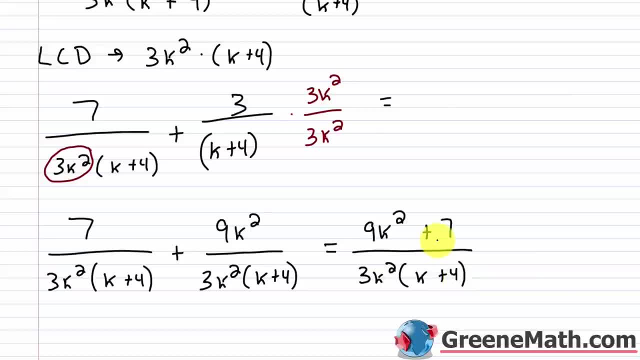 This numerator here is prime there's nothing I can really pull out so I'm not going to be able to really cancel anything here. 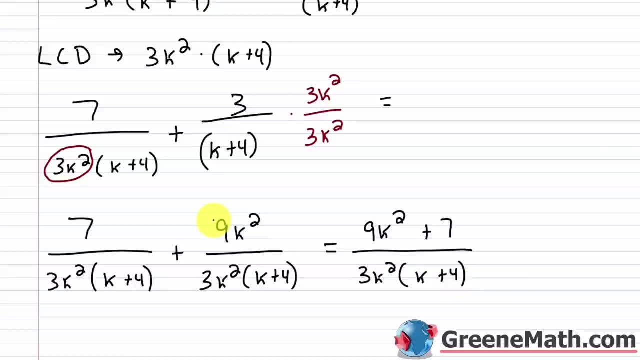 Again don't make the mistake that I see so many students do. 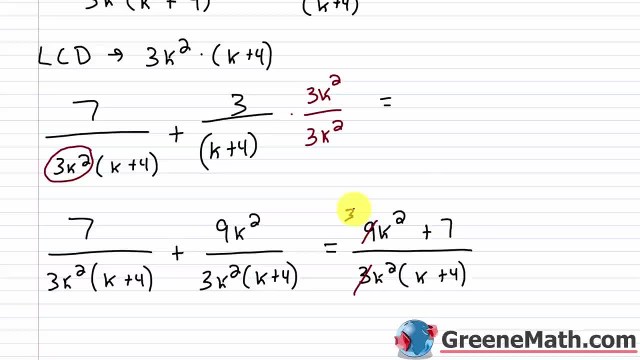 They'll go okay well this 9 can cancel with this 3 and this is a 3. No that doesn't work like that. You cancel common factors. This is not 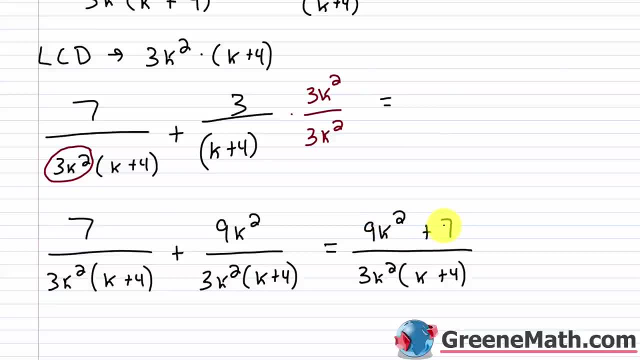 a factor. This is 9k squared plus 7 so you can't cancel there. 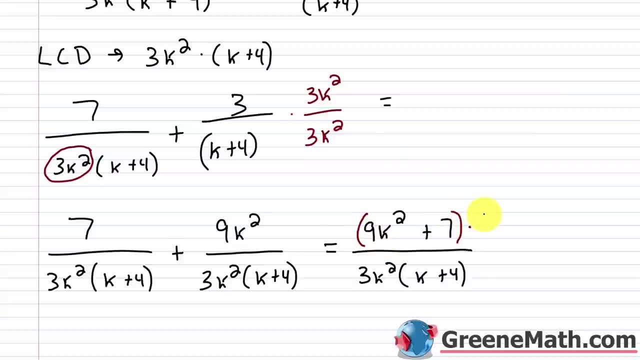 If I had this being multiplied by let's say 9k squared something like that well yeah since this is multiplication here these are factors. 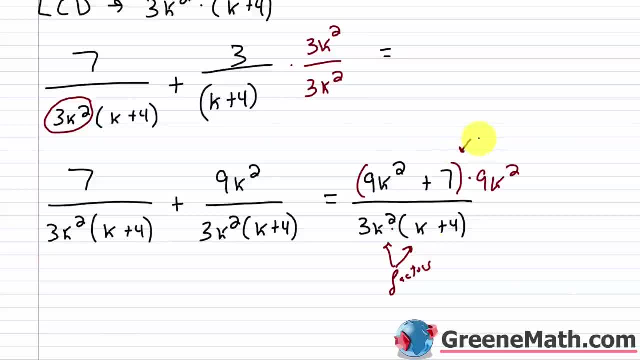 These are factors and then these would be factors if that's the problem that I had so then I could cancel this 9 with this 3 and this would give me a 3 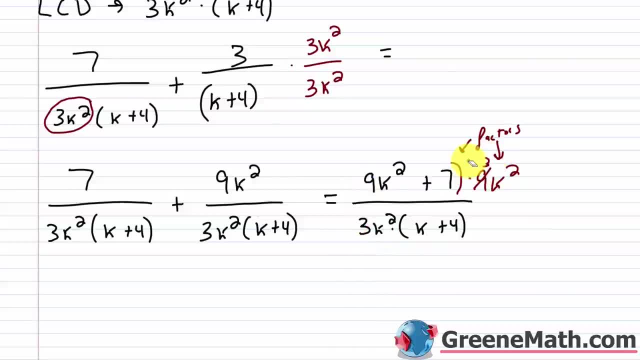 if that's the problem we have. We don't have that though so there's nothing I can do to simplify. Let me erase all this. There's nothing I can do to simplify it so 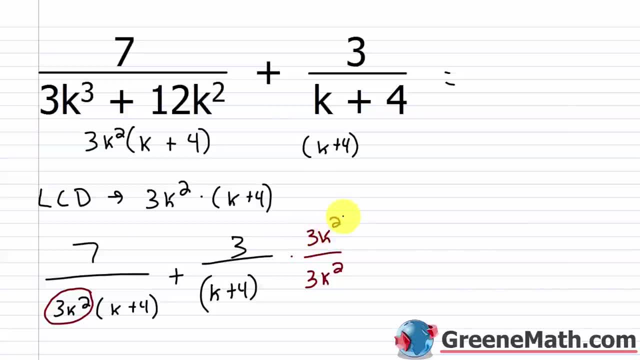 3k squared over 3k squared is 1.. Just a complicated form of 1, but it's still 1.. Now if I multiply here 3 times 3k squared is 9k squared. Let's scroll down a little bit. 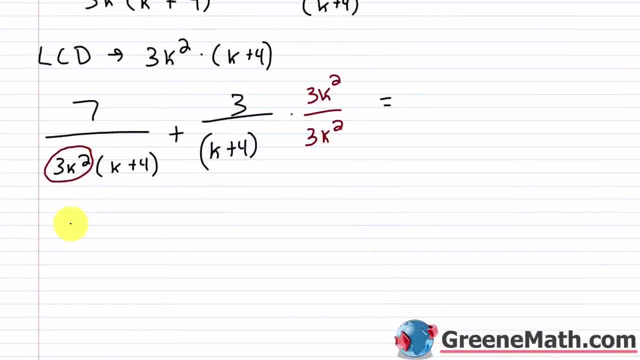 So this equals- I'll rewrite this first- 7, over again 3k squared times the quantity k plus 4.. As I just said, 3 times 3k squared is 9k squared, And this is over 3k squared times the quantity k plus 4.. 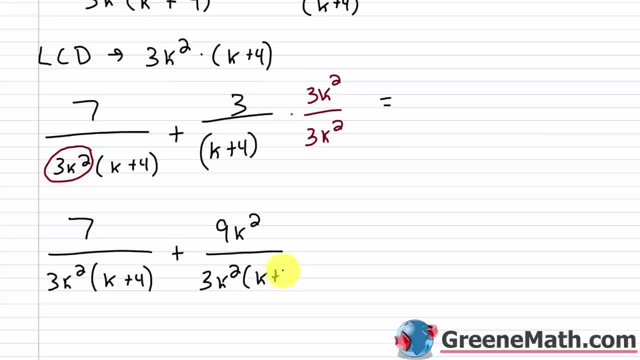 So 3k squared times the quantity k plus 4.. So now I have a common denominator. This denominator is the same as this denominator, So I can just add the numerators, And so basically what I'd have is just 9k squared plus 7 over that common denominator. 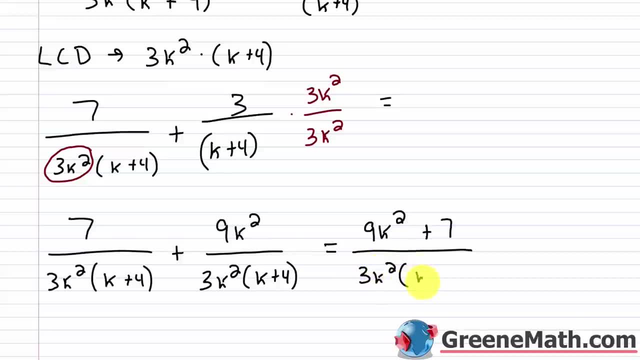 Of 3k squared times the quantity k plus 4.. And in this particular case there's nothing I can do to simplify This numerator. here is prime. There's nothing I can really pull out, So I'm not going to be able to really cancel anything here. 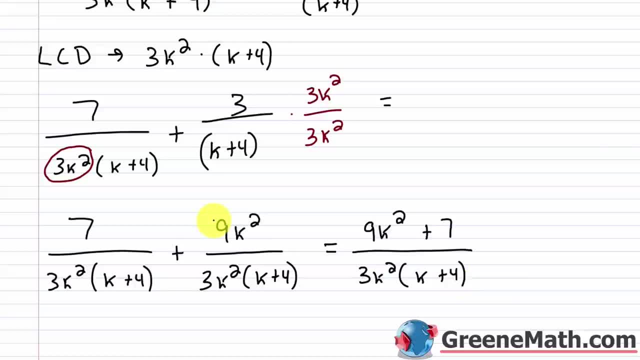 Again, don't make the mistake that I see so many students do. They'll go okay. well, this 9 can cancel with this 3 and this is a 3.. No, that doesn't work like that. You cancel common factors. 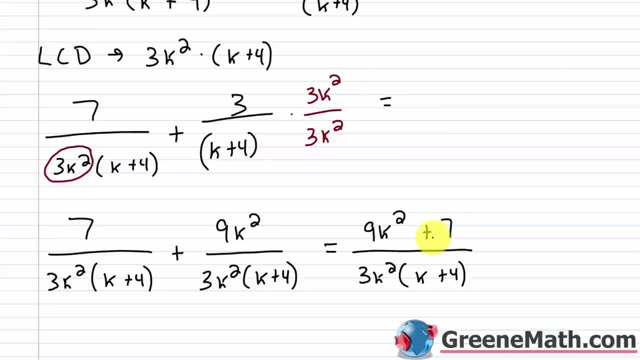 This is not a factor. This is 9k squared plus 7.. So you can't cancel there. If I had this being multiplied by, let's say, 9k squared something like that, Well, yeah, since this is multiplication here, these are factors. 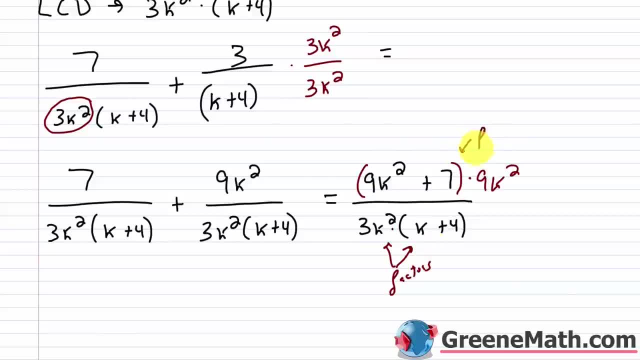 These are factors, And then these would be factors if that's the problem that I had, So then I could cancel this 9 with this 3.. And this would give me a 3 if that's the problem we have. We don't have that, though. 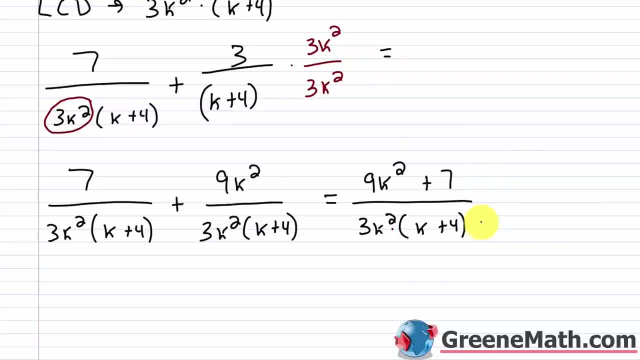 So there's nothing I can do to simplify. Let me erase all this. There's nothing I can do to simplify it. So 9k squared plus 7 over 3k squared times, the quantity k plus 4 is our simplified answer. 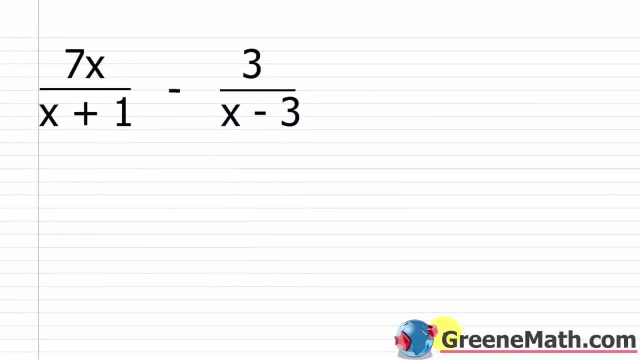 Okay, let's take a look at another one. So we have 7x over x plus 1. And we're subtracting away 3 over x minus 3. So the LCD here is very, very simple. Each of these is prime right. 9k squared plus 7 over 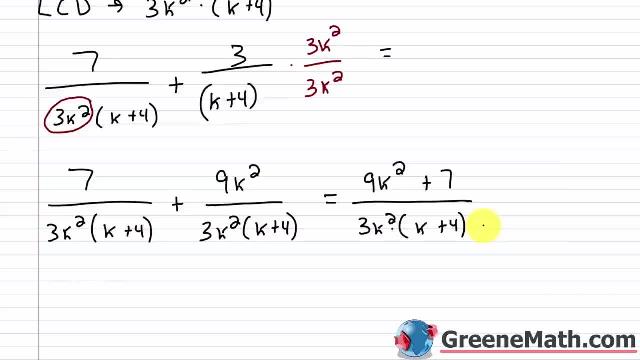 3k squared times the quantity k plus 4 is our simplified 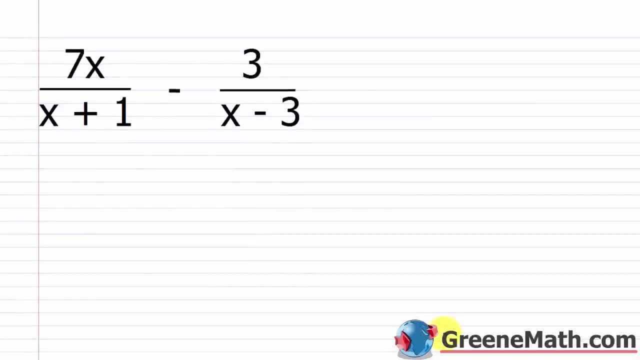 answer. Okay let's take a look at it so we have 7x over x plus 1 and we're subtracting 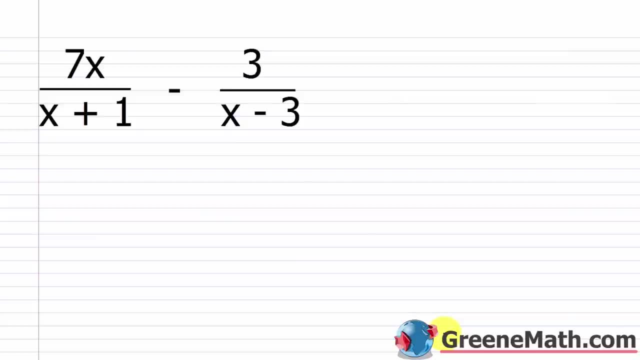 away 3 over x minus 3 so the LCD here is very very simple each of these is prime right so I can't factor x plus 1 and I can't factor x minus 3 so I just multiply the two together to get 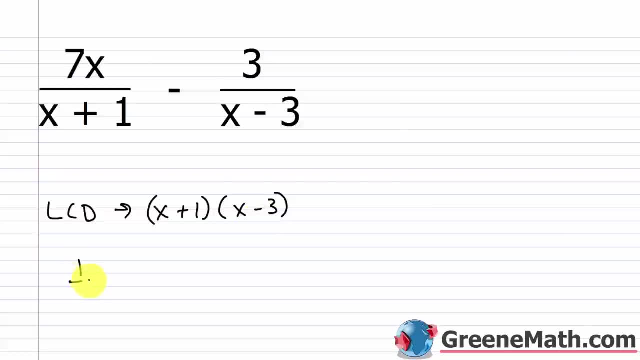 the LCD. It's just like if I had fractions where I had 1 fifth 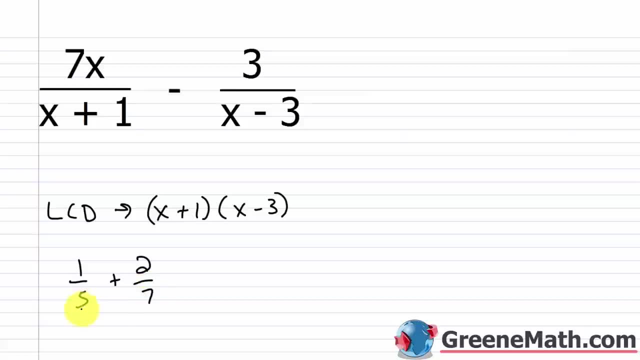 plus let's say 2 sevenths right each of these is prime so to get the LCD I'd just multiply 5 times 7 and I get 35. Well same thing here each is prime multiply the two together to get the LCD. Alright 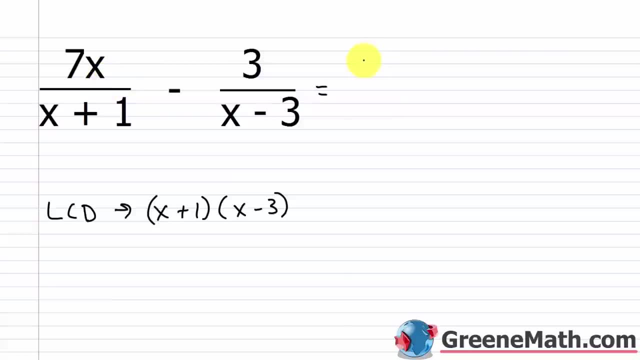 so in order to change 7x over x plus 1 into a rational expression with this as it's denominator I need to multiply by what? I'm missing an x minus 3 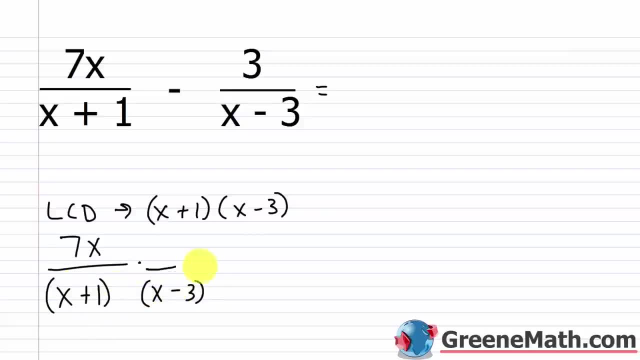 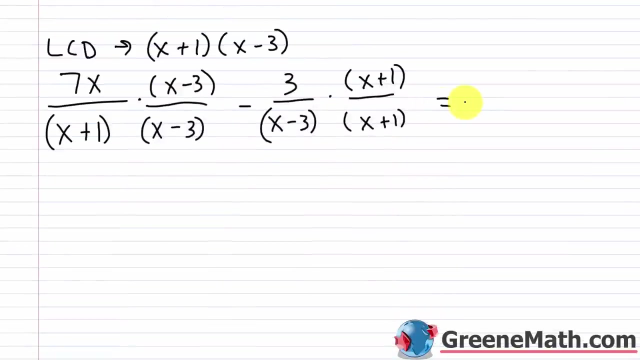 so an x minus 3 is going down here and so I've got to also do that to the numerator so that it's legal then minus up here I have a 3 over x minus 3 and what I'm missing here is the x plus 1 so I'm going to multiply by I have x plus 1 down here and again to make it legal I multiply by x plus 1 up here so now if we crank this out what I'm going to get is 7x times x is 7x squared 7x times negative 3 is 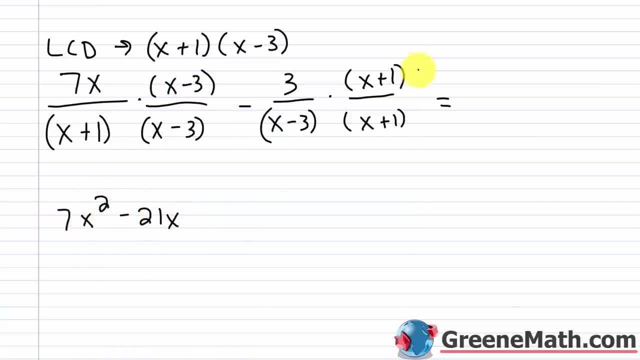 minus 21x and then I'm subtracting away this right here so 3 times x is 3x 3 times 1 is 3 so plus 3 now again I'm subtracting all of this away so I'm going to put minus and I'm going to put parentheses around this and what that's going to tell me is that to remove the parentheses again I've got to change the sign of each term so don't make the mistake again of just putting minus 3x plus 3 both of those need to have their signs changed so this is going to be 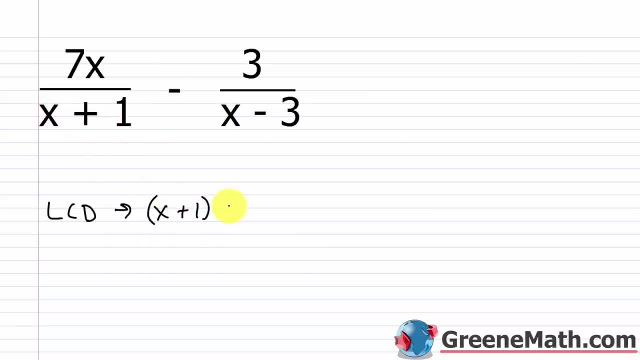 So I can't factor x plus 1.. And I can't factor x minus 3.. So I just multiply the two together to get the LCD. It's just like if I had fractions where I had 1 fifth plus, let's say, 2 sevenths. 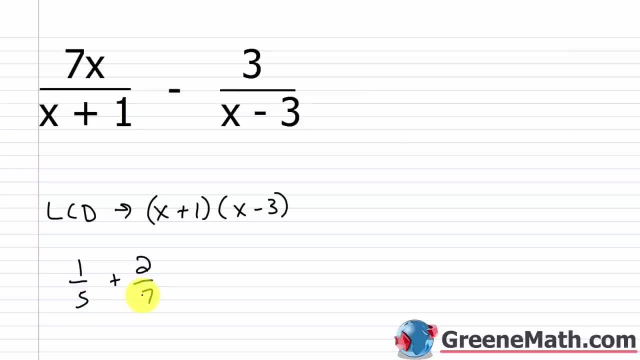 Right, Each of these is prime. So to get the LCD, I just multiply 5 times 7, and I get 35.. Well, same thing here. Each is prime. Multiply the two together to get the LCD, All right. 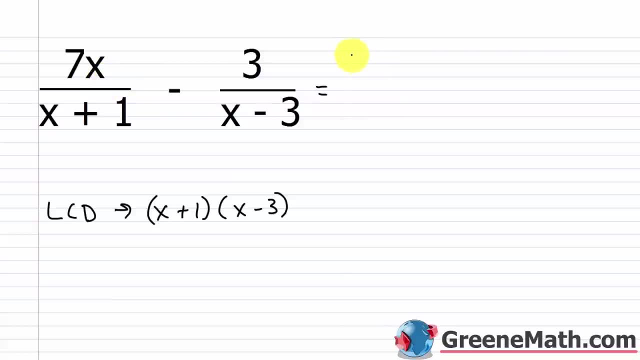 So in order to change 7x over x plus 1 into a rational expression with this as its denominator, I need to multiply by what I'm missing: an x minus 3.. So an x minus 3 is going down here, And so I've got to also do that to the numerator so that it's legal. 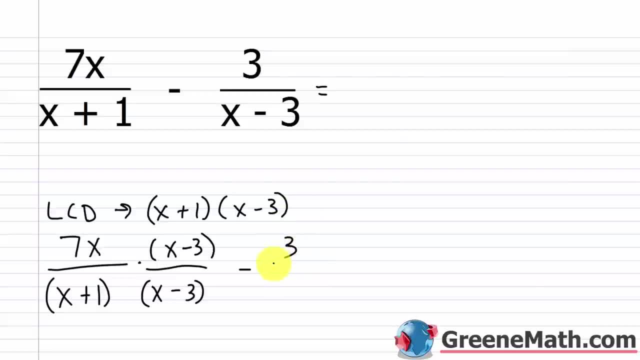 Then minus Up here I have a 3 over x minus 3.. And what I'm missing here is the x plus 1.. So I'm going to multiply by. I have x plus 1 down here And again, to make it legal, I multiply by x plus 1 up here. 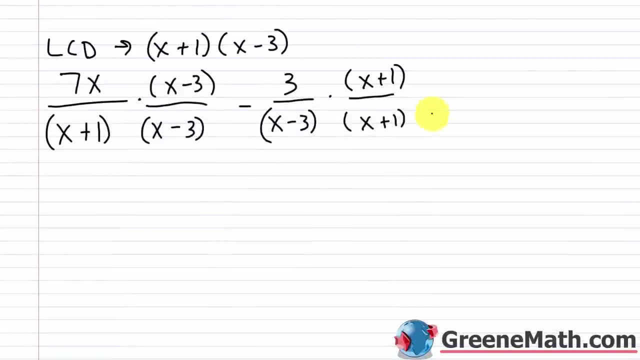 So now, if we crank this out, what I'm going to get is 7x times x. 7x times x is 7x squared, 7x times negative 3 is minus 21x, And then I'm subtracting away this right here. 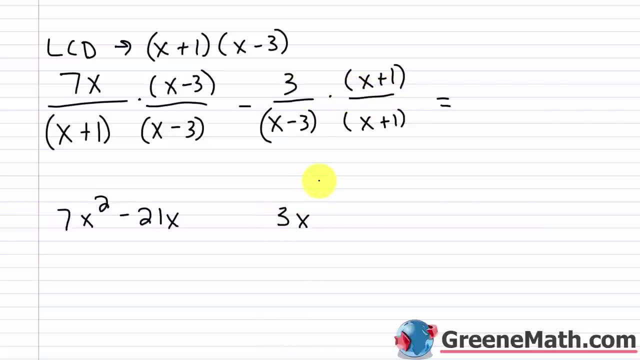 So 3 times x is 3x, 3 times 1 is 3.. So plus 3.. Now again, I'm subtracting all of this away, So I'm going to put minus and I'm going to put parentheses around this. 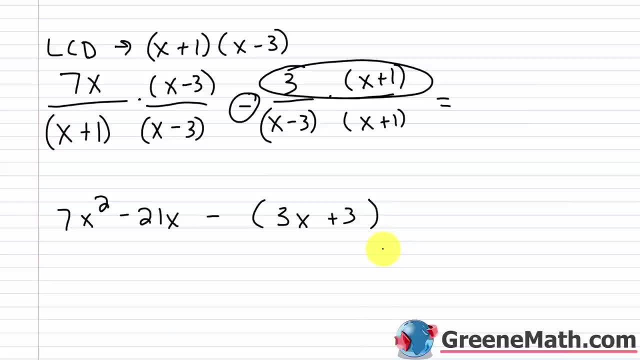 And what that's going to tell me is that, to remove the parentheses again, I've got to change the sign of each term. So don't make the mistake again of just putting minus 3x plus 3.. Both of those need to have their signs changed. 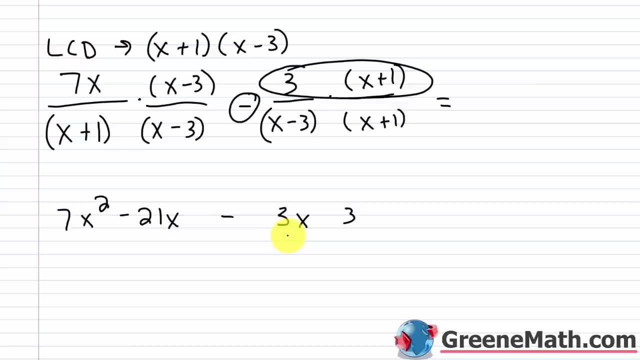 So this is going to be minus 3x changes from positive to negative, And then minus 3, again changes from positive to negative. So this is over the common denominator of x plus 1.. That quantity times x minus 3.. 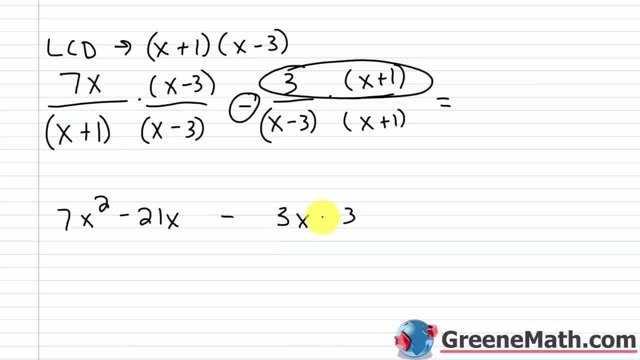 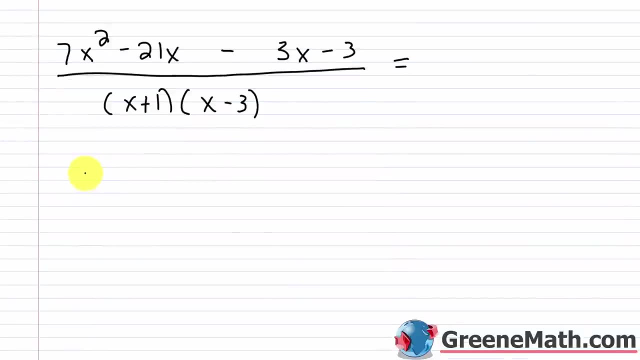 minus 3x changes from positive to negative and then minus 3 again changes from positive to negative so this is over the common denominator of x plus 1 that quantity times x minus 3 and now we just want to combine like terms so 7x squared nothing I can do with that negative 21x minus 3x is minus 24x and then minus 3 and this is over the quantity again x plus 1 times x 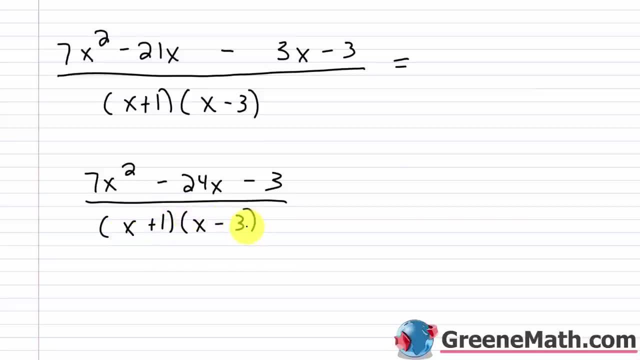 minus 3 now here comes part of 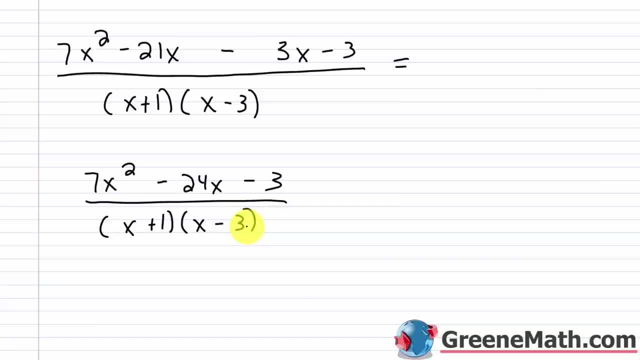 the problem sometimes you're going to get something like this and it's going to be extremely tedious right so I've gone through all that work and now I've got to factor this to see if I'll have a common factor with the denominator to simplify 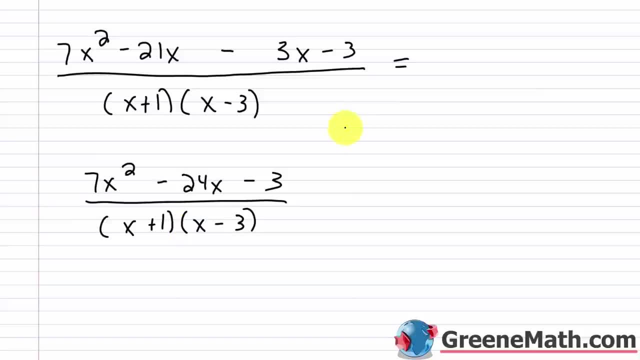 so I've got to think about two integers whose product so I want a product of what 7 times negative 3 so of negative 21 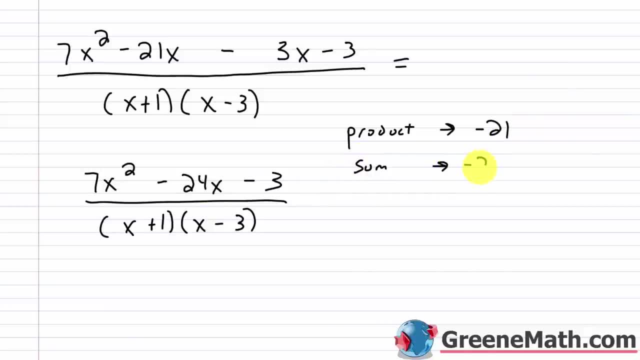 and then whose sum is going to be negative 24 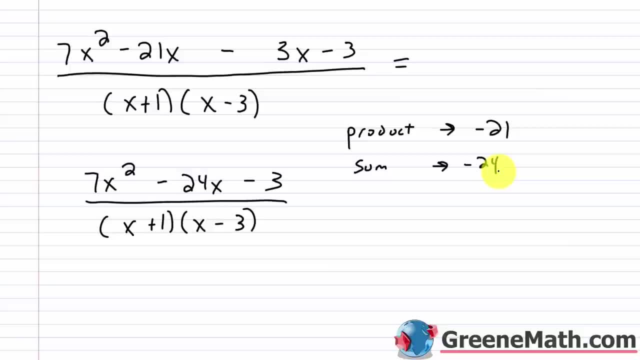 now for 21 you basically only have what you have 1 times 21 and you have 3 times 7 that's it I can't play with 1 and 21 I can't play with the signs and make that sum to negative 24 I also can't play with the signs with 3 and 7 and make that sum to negative 24 so this is a prime polynomial 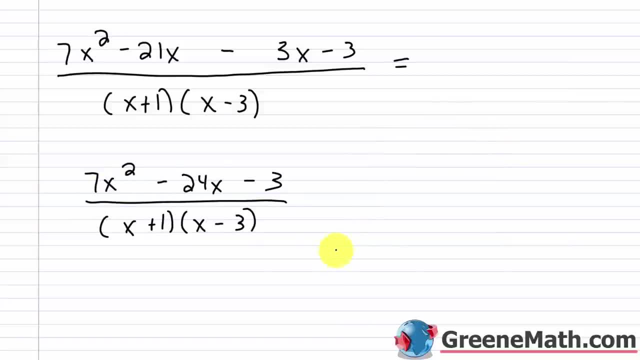 up here in the numerator I can't factor it and so what I'm going to say here is that this is simplified we have 7x squared minus 24x minus 3 over the quantity x 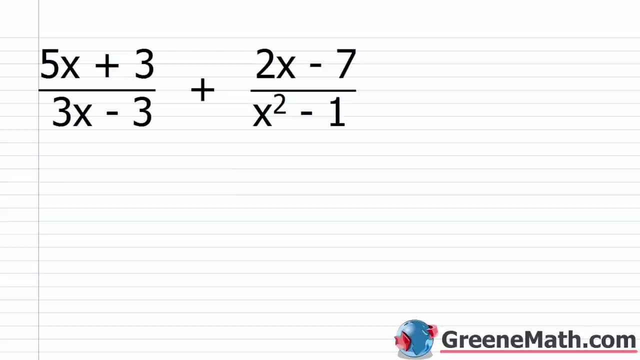 plus 1 times the quantity x minus 3 alright let's take a look at another one so we have 5x plus 3 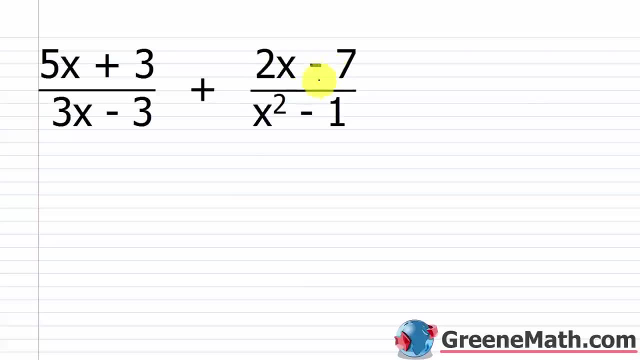 over 3x minus 3 and we're adding to this 2x minus 7 over x squared minus 1 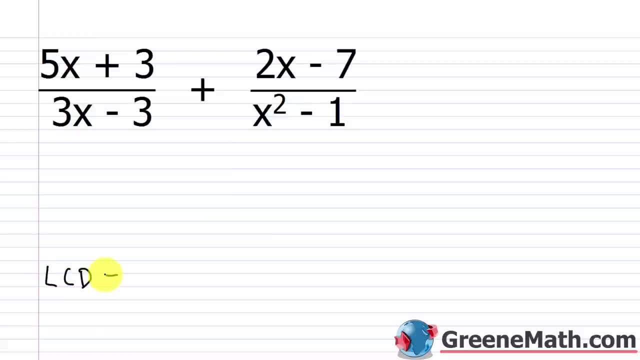 so again to find the LCD I want to factor the denominators for this one I could pull out a 3 so I would have 3 times I would have x minus 1 x minus 1 for here it's the difference of 2 squares so some of these you should start to remember like x squared minus 1 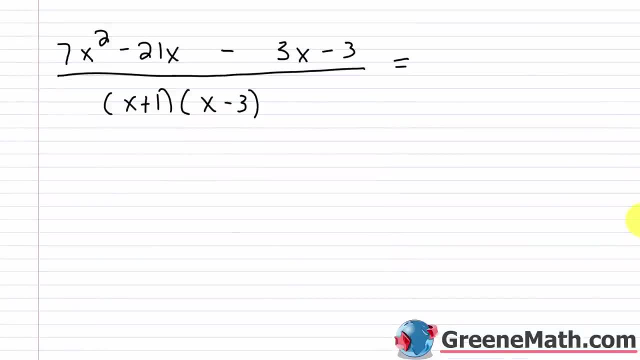 And now we just want to combine like terms. So 7x squared. nothing I can do with that Negative 21x minus 3x is minus 24x And then minus 3.. And this is over the quantity. again x plus 1 times x minus 3.. 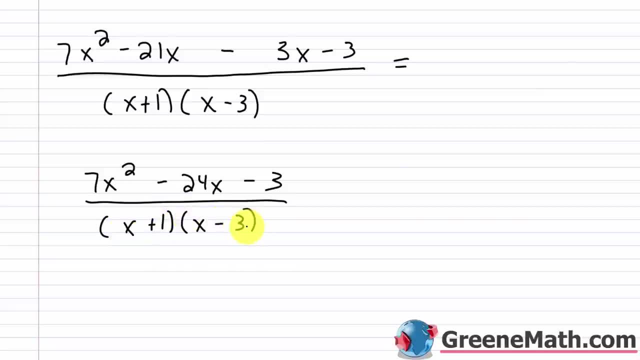 Now here comes part of the problem. Sometimes you're going to get something like this and it's going to be extremely tedious, right? So I've gone through all that work and now I've got to factor this to see if I'll have a common factor with the denominator to simplify. 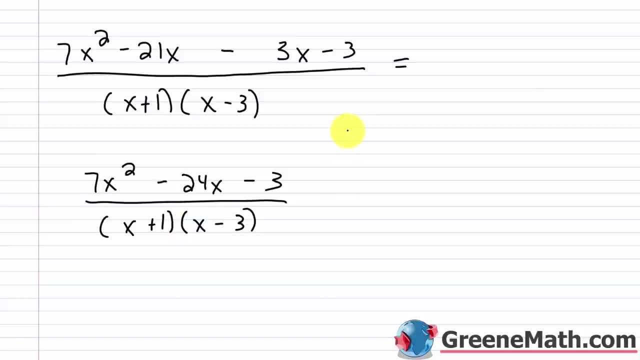 So I've got to think about two integers. whose product? so I want a product of what? 7 times negative 3. So of negative 21. And then whose sum is going to be negative 24. Now for 21,. you basically only have what. 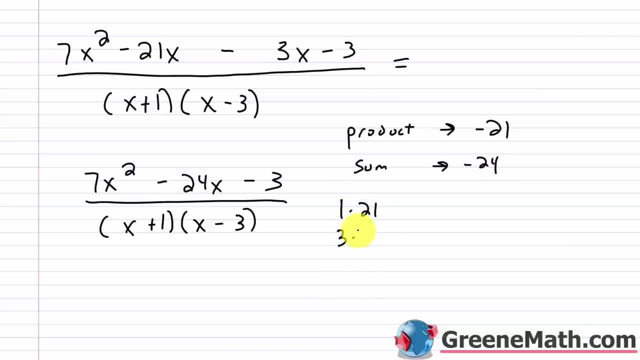 You have 1 times 21, and you have 3 times 7.. That's it. I can't play with 1 and 21.. I can't play with the signs and make that sum to negative 24.. I also can't play with the signs with 3 and 7 and make that sum to negative 24.. 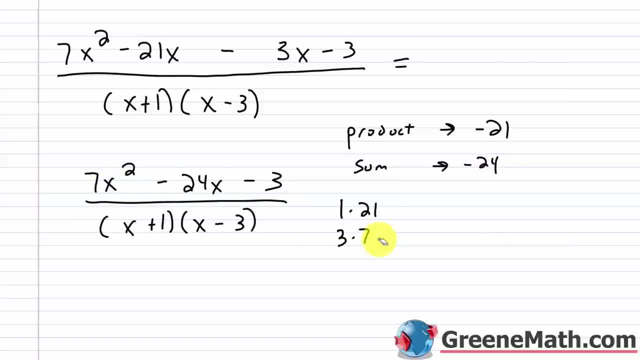 So this is a prime polynomial up here in the numerator, I can't factor it, And so what I'm going to say here is that this is simplified. We have 7x squared minus 24x minus 3 over the quantity x plus 1 times the quantity x minus 3.. 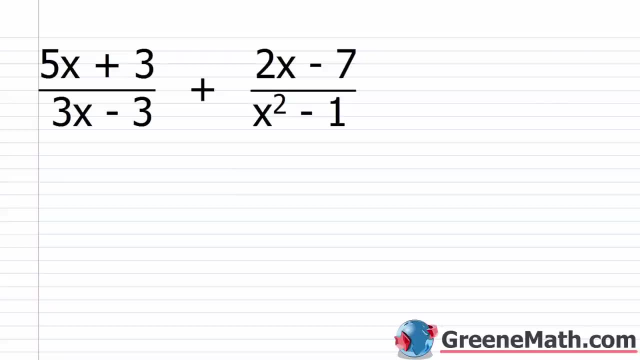 All right, let's take a look at another one. So we have 5x plus 3 over 3x minus 3.. Then we're adding to this 2x minus 7 over x squared minus 1.. So again to find the LCD, I want to factor the denominators. 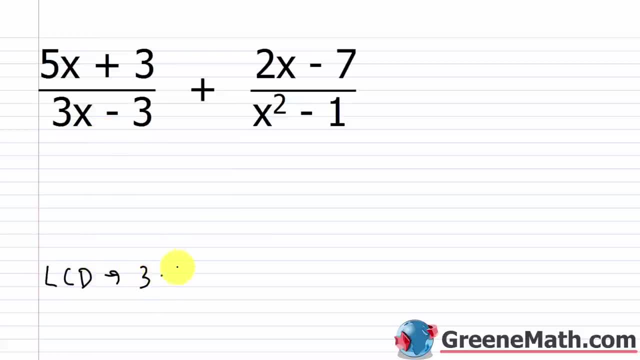 For this one I could pull out a 3.. So I would have 3 times. I would have x minus 1.. x minus 1.. For here it's the difference of two squares. So some of these you should start to remember, like x squared minus 1, x squared minus 4,. 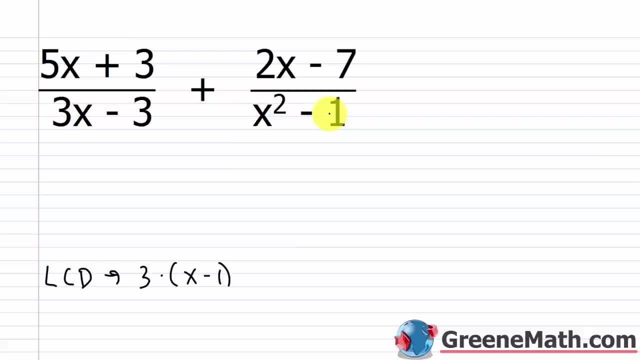 you know things like that: x squared minus 16.. Start to memorize these because as they come up, you want to be able to see that. okay, if I see a binomial here and I got a minus sign, first guy is squared. 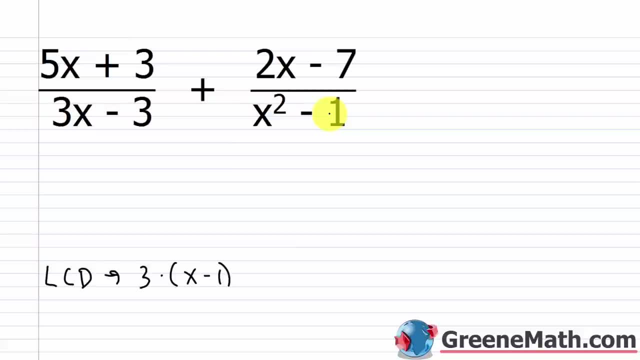 x squared minus 4 you know things like that x squared minus 16 start to memorize these because as they come up you want to be able to see that okay if I see a binomial here and I got a minus sign first guy is squared the second guy is a perfect square I know I have the difference of 2 squares so x squared minus 1 will factor into x plus 1 times x minus 1 now I've already got an x minus 1 here so I don't need to put it into the list of the LCD what I do need to do is throw in this x plus 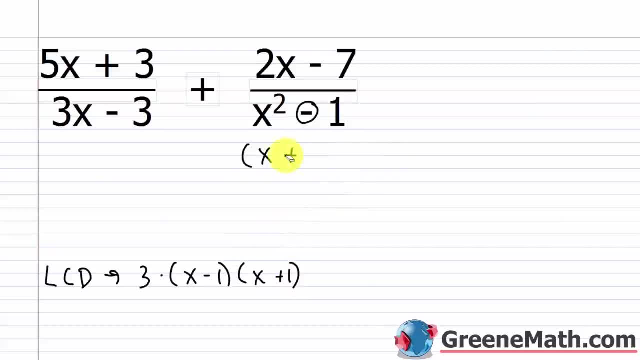 1 because it's not currently present so my LCD will be 3 times the quantity x minus 1 times the quantity x plus 1 so let's go ahead and change each rational expression to an equivalent rational expression where the LCD here is its denominator so I'll have 5x plus 3 over I'm going to write this as 3 times the quantity x minus 1 and what I'm missing here is this x plus 1 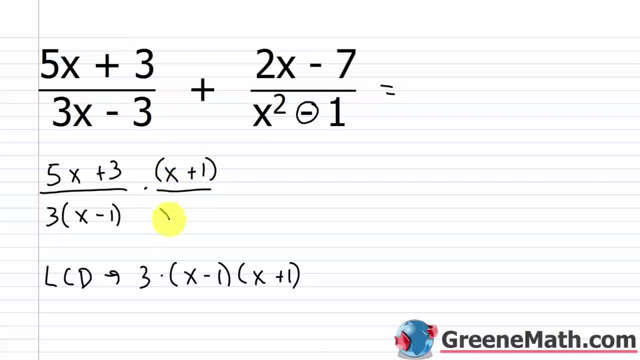 so I'm going to multiply by x plus 1 over x plus 1 then plus over here I have 2x minus 7 over I have x plus 1 times x minus 1 those two quantities I'm missing a 3 here so times 3 over 3 now very important since I'm multiplying by 3 remember to use parentheses don't just multiply 3 times 2x and be done so I'm going to put parentheses around it because I've got to use my distributive property okay so let's put equals 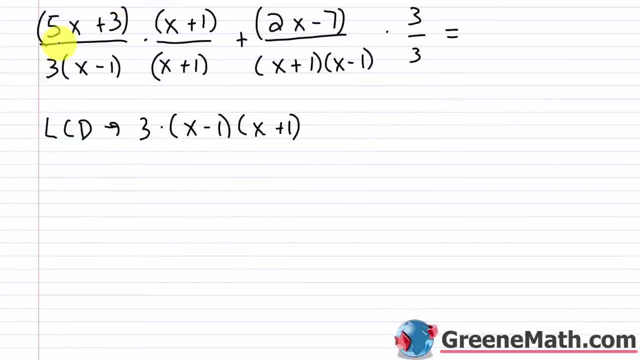 here let's scroll down and get some room going and so I'm going to use FOIL here 5x times 2x is 5x squared the outer 5x times 1 is 5x the inner 3 times x is 3x so 5x plus 3x is 8x so plus 8x and then the last 3 times 1 is 3 so plus 3 and plus again use your distributive property 3 times 2x is 6x then minus 3 times 7 that's 21 okay so this is all 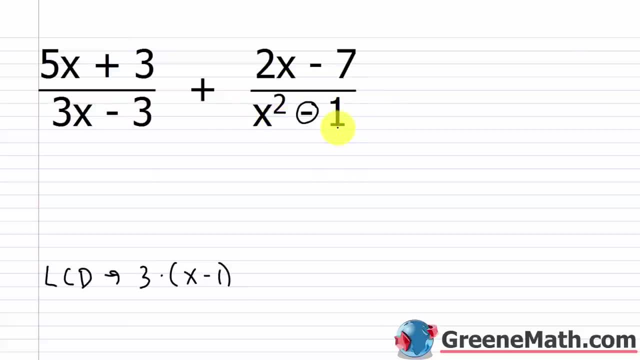 The second guy is a perfect square. I know I have the difference of two squares, So x squared minus 1 will factor into x plus 1.. Times, x minus 1.. Now I've already got an x minus 1 here, So I don't need to put it into the list of the LCD. 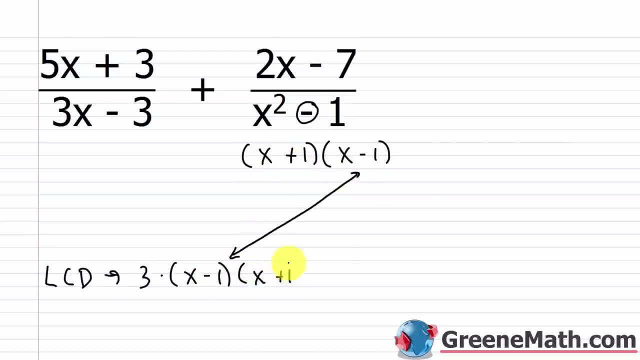 What I do need to do is throw in this x plus 1, because it's not currently present. So my LCD will be 3 times the quantity x minus 1 times the quantity x plus 1.. So let's go ahead and change each rational expression to an equivalent rational expression. 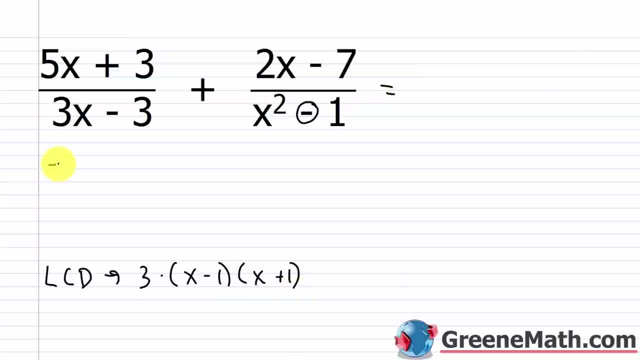 where the LCD here is its denominator. So I'll have 5x. So I'll have 5x plus 3 over. I'm going to write this as 3 times the quantity x minus 1.. And what I'm missing here is this: x plus 1.. 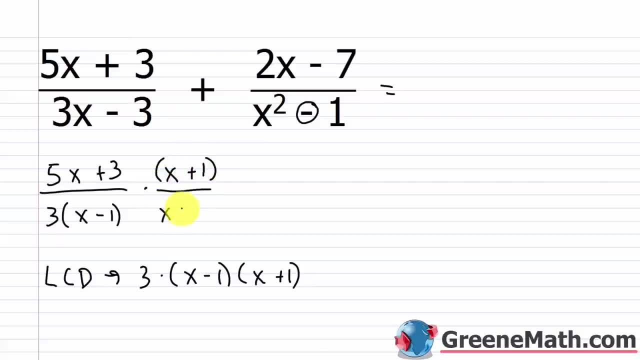 So I'm going to multiply by x plus 1 over x plus 1.. Then plus over here I have 2x minus 7 over I have x plus 1 times x minus 1.. Those two quantities. I'm missing a 3 here. 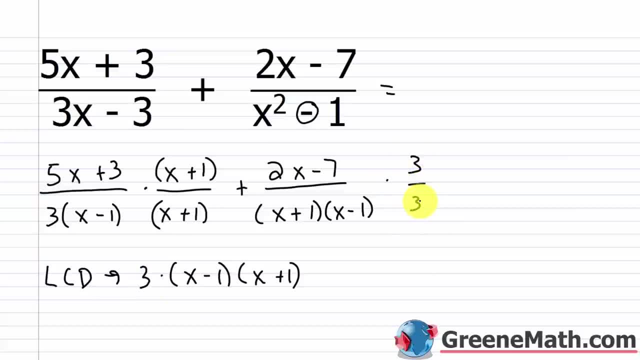 So times 3 over 3.. Now This is important, since I'm multiplying by 3.. Remember to use parentheses. Don't just multiply 3 times 2x and be done. So I'm going to put parentheses around it because I've got to use my distributive property. 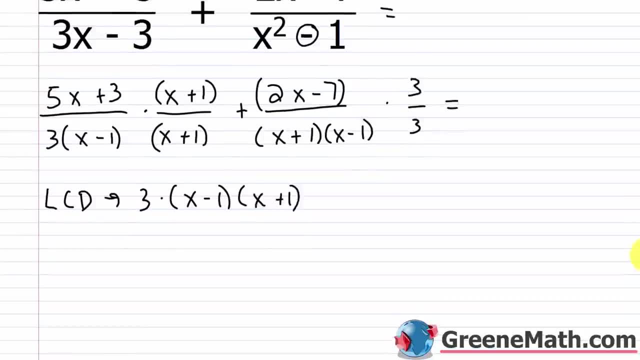 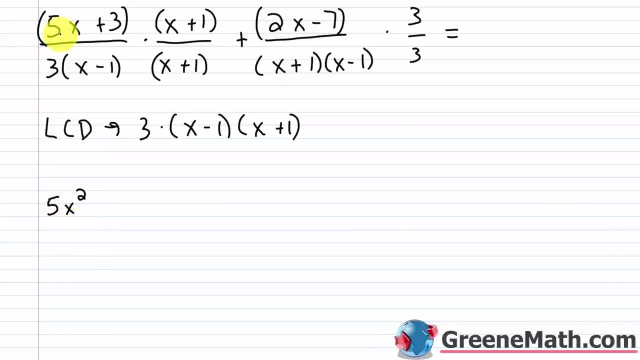 Okay, So let's put equals here, Let's scroll down and get some room going, And so I'm going to use FOIL here. 5x times x is 5x squared. The outer 5x times 1 is 5x. 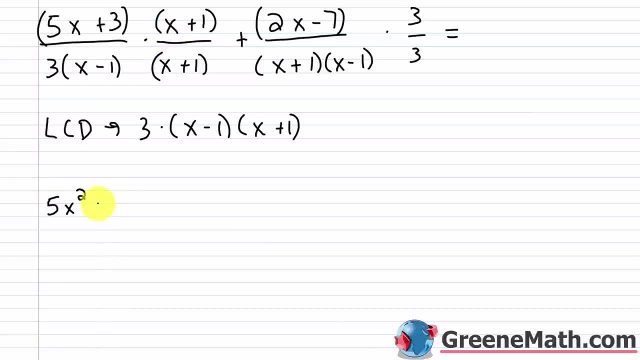 The inner 3 times x is 3x, So 5x plus 3x is 8x, So plus 8x. And then the last 3 times 1 is 3.. So plus 3.. Then plus. 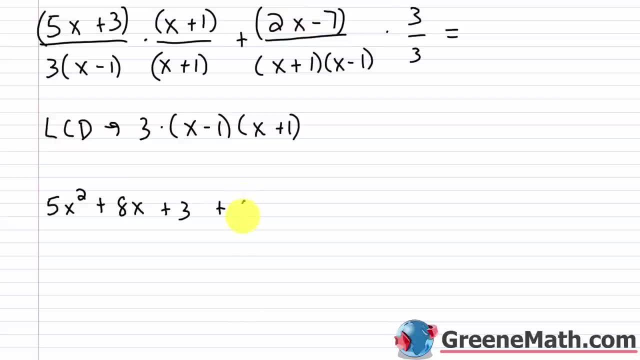 Again, use your distributive property 3 times 2x is 6x, Then minus 3 times 7.. That's 21.. Okay, So this is all over that common denominator of 3 times the quantity x plus 1 times the quantity x minus 1.. 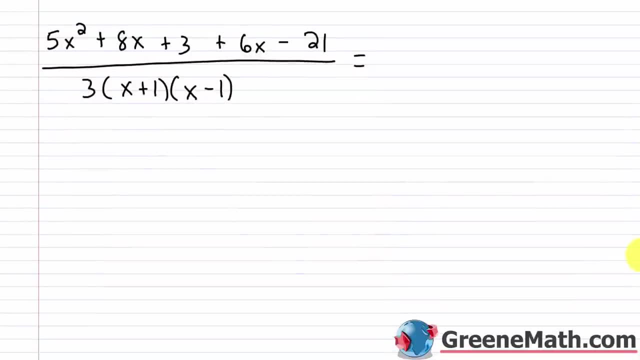 So now let's go ahead and simplify the numerator. We'll have 5x squared. Nothing I can do with that. I have 8x plus 6x, That's 14x, And then I have 3 and negative 21.. 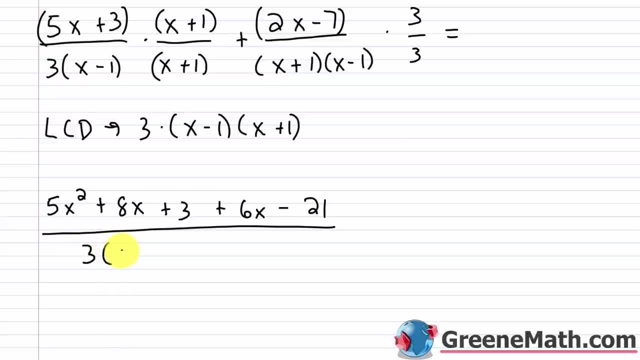 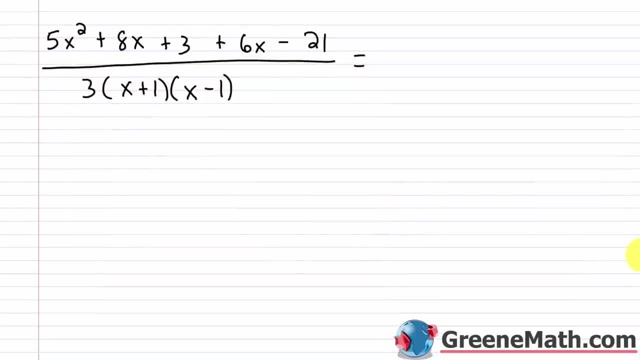 over that common denominator of 3 times the quantity x plus 1 times the quantity x minus 1 so now let's go ahead and simplify the numerator we'll have 5x squared nothing I can do with that I have 8x plus 6x that's 14x so plus 14x and then I have 3 and negative 21 that's minus 18 so 5x squared plus 14x minus 18 and again this is over that common denominator of 3 times the quantity 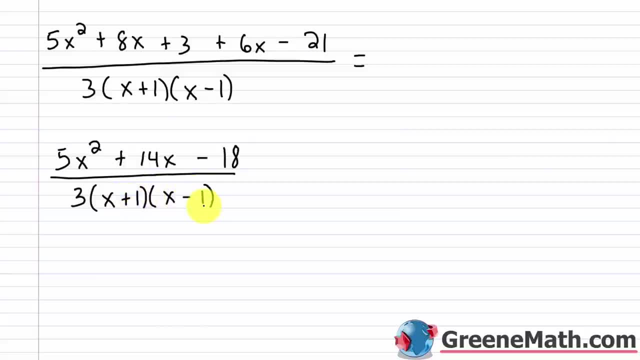 x plus 1 times the quantity x minus 1 now can I factor this trinomial 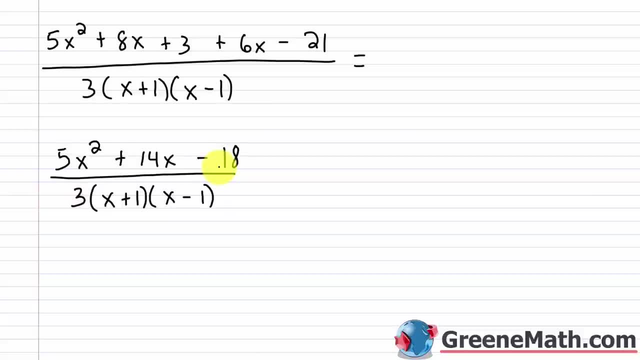 in the numerator so 5 times negative 18 is negative 90 so give me two integers whose product product is negative 90 and whose sum is 14 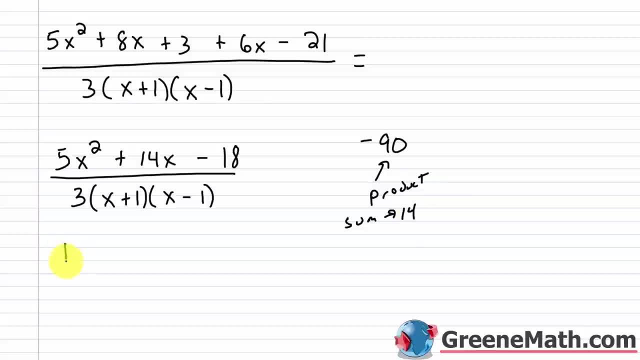 well let me think about that I've got what I've got 1 times 90 that won't work I've got 2 times 45 not going to work I've got 3 times 30 I've got not divisible by 4 I've got 5 times 18 that won't work I've got 6 times 15 that won't work 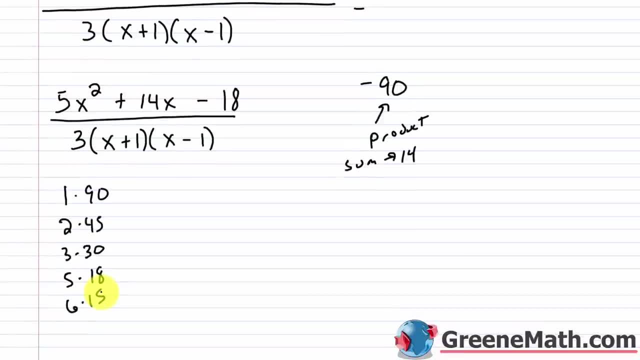 not divisible by 7 not divisible by 8 is divisible by 9 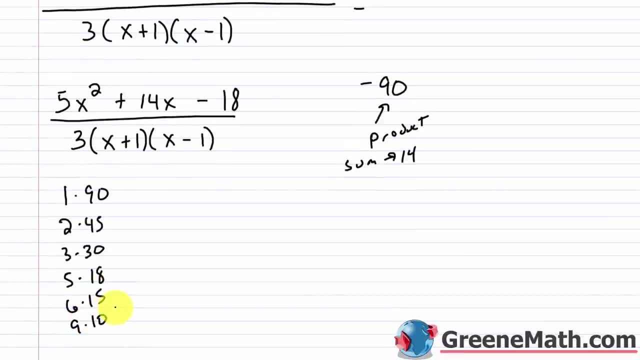 it's going to be 9 times 10 and that's all we can really do so I can't take 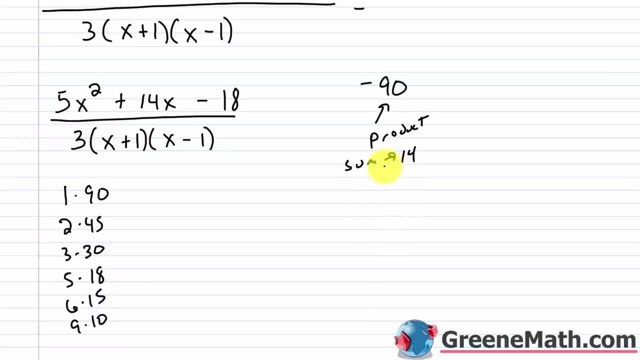 any of these and manipulate the signs to get a sum of 14 and a product of negative 90 so this 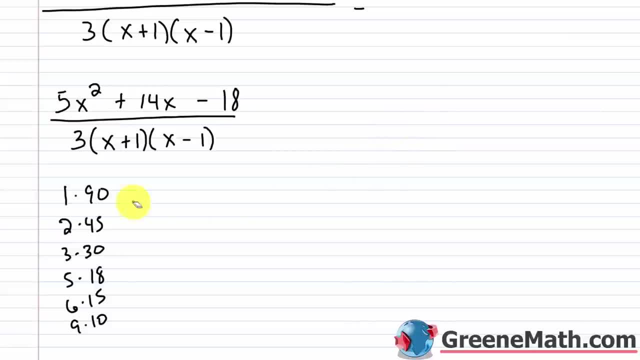 trinomial up here is going to be prime and I can't factor it so 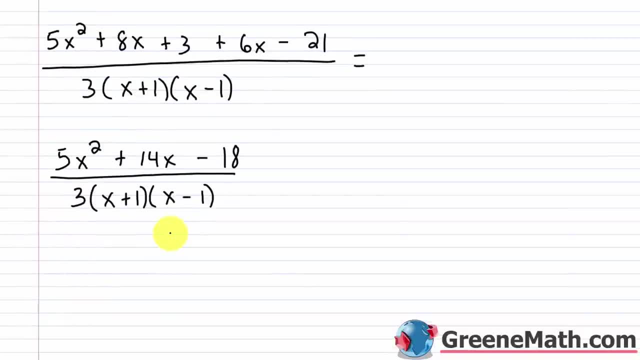 what's going to happen is I'm just going to leave my answer as it is this is simplified 5x squared plus 14x minus 18 over 3 times the quantity x plus 1 times the quantity x minus 1 alright let's take a look at another one 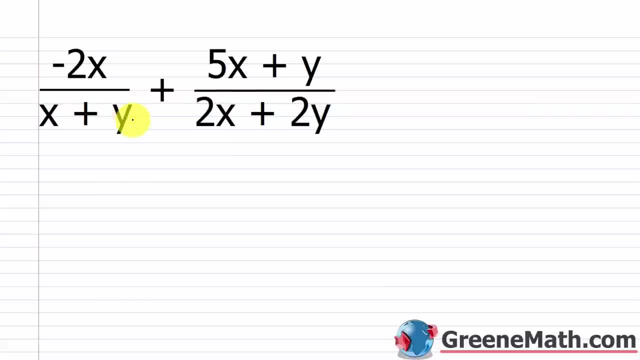 let's say I have negative 2x over x plus y then I'm adding to this 5x plus y 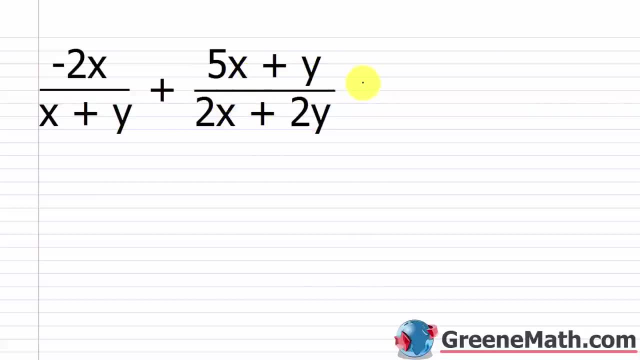 over 2x plus 2y so what I want to do here again is start out by finding the LCD so it's the LCD 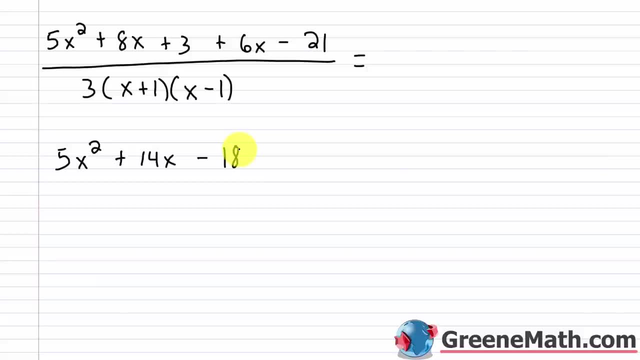 That's minus 18.. So 5x squared plus 14x minus 18.. And again, this is over that common denominator of 3 times the quantity x plus 1 times the quantity x minus 1.. Now can I factor this trinomial in the numerator? 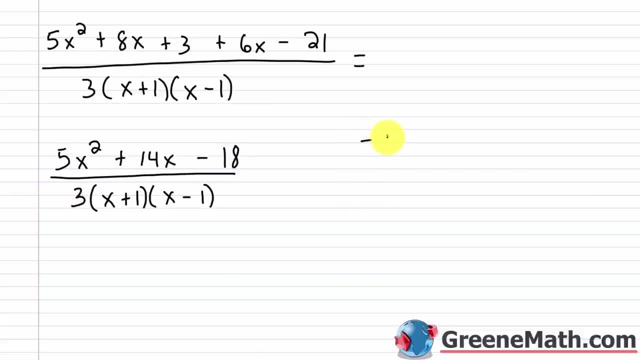 So 5 times negative 18 is negative 90.. So give me two integers whose product is negative 90. And whose sum is 14.. Well, let me think about that. I've got what I've got 1 times 90.. 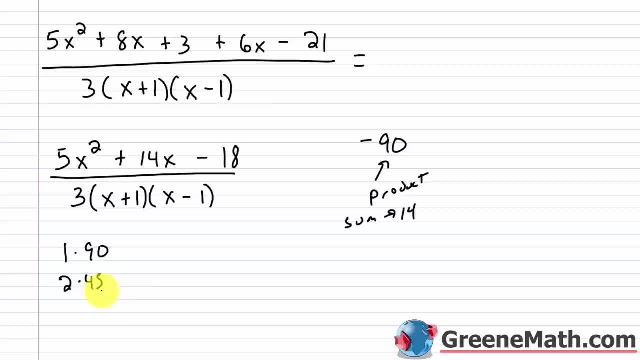 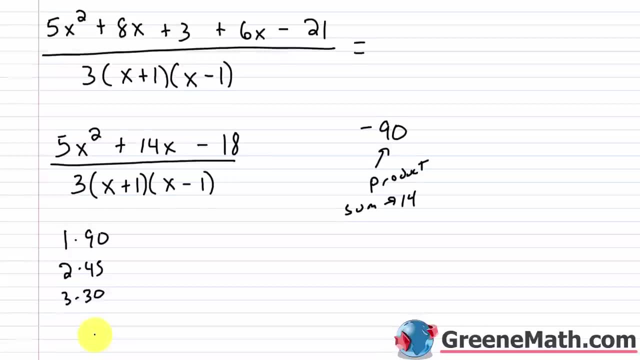 That won't work. I've got 2 times 45.. Not going to work. I've got 3 times 30.. I've got not divisible by 4.. I've got 5 times 18.. That won't work. 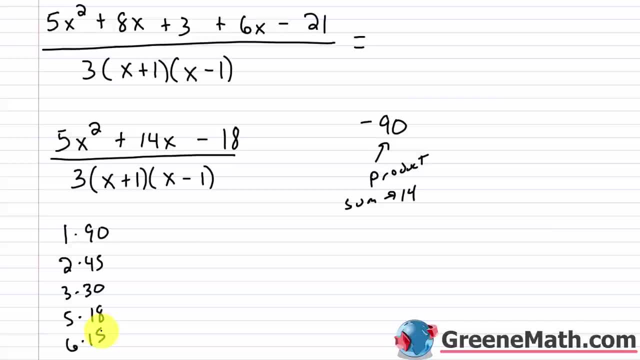 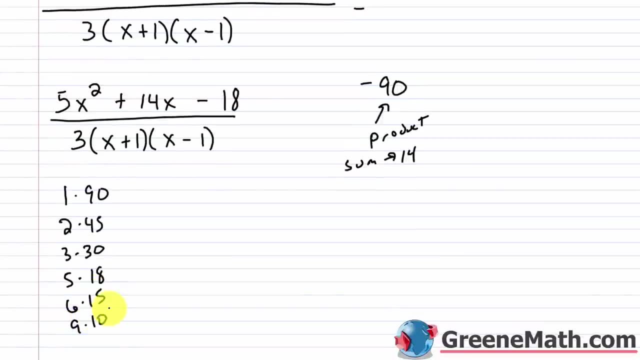 I've got 6 times 15.. That won't work. Not divisible by 7.. Not divisible by 8. Is divisible by 9. It's going to be 9 times 10. And that's all we can really do. 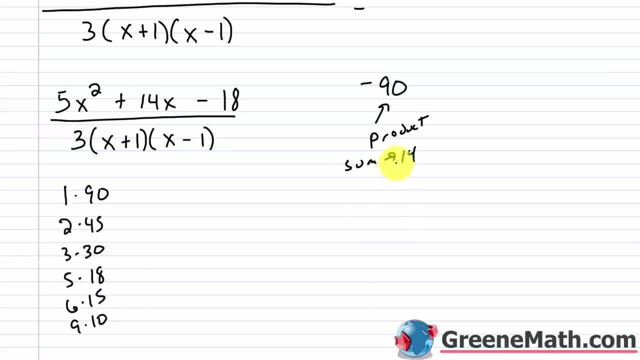 So I can't take any of these and manipulate the signs to get a sum of 14 and a product of negative 90. So this trinomial up here is going to be prime And I can't factor it. So what's going to happen is I'm just going to leave my answer as it is. 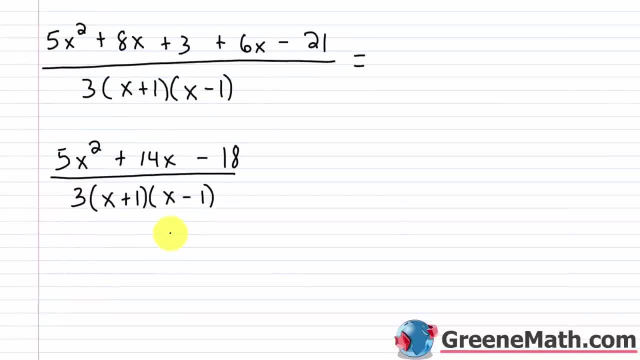 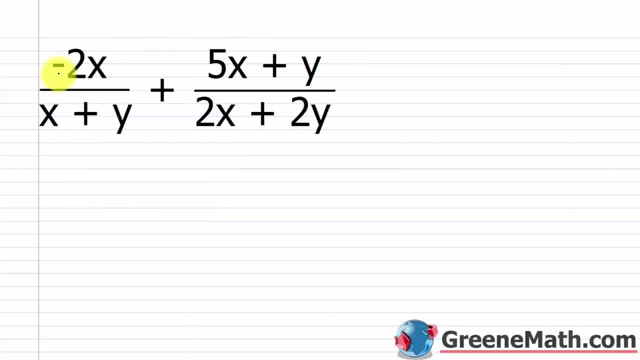 This is simplified: 5x squared plus 14x minus 18, over 3 times the quantity x plus 1 times the quantity x minus 1.. All right, Let's take a look at another one. Let's say I have negative 2x over x plus y. 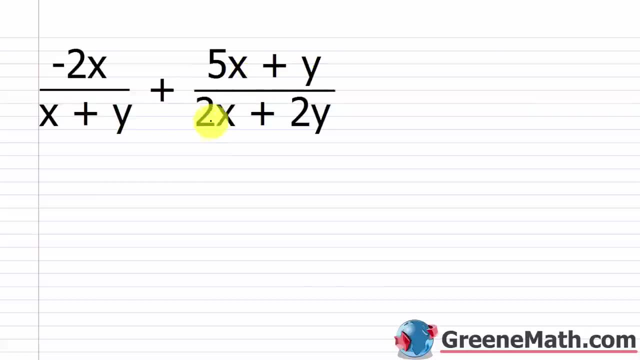 Then I'm adding to this 5x plus y over 2x plus 2y. So what I want to do here again is start out by finding the LCD. So it's the LCD, This x plus y. I can't factor that. 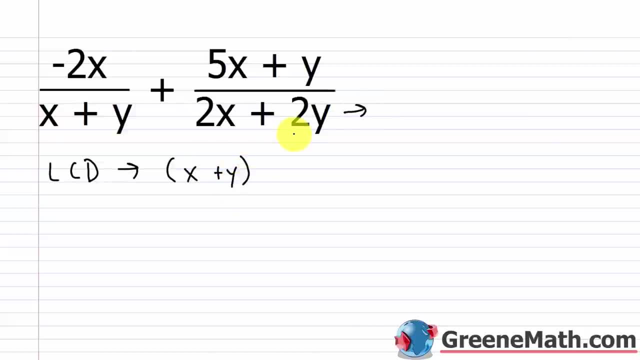 Over here I can factor out a 2. So I could write this as 2 times the quantity x plus y. Now I've already got an x plus y here, I just need the 2.. So the LCD is 2 times the quantity x plus y. 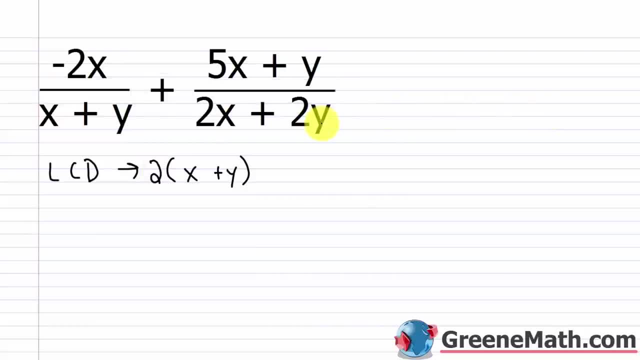 So, because this denominator is already the LCD, I don't need to change this rational expression, I just need to change the one on the left. So what I'm going to do, I'm going to multiply negative 2x over x plus y times. what I'm missing here is a 2.. 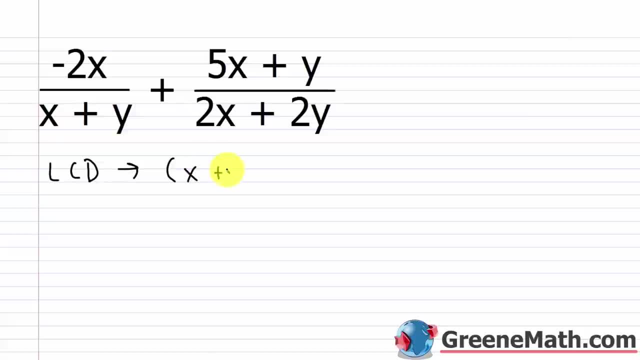 this x plus y I can't factor that 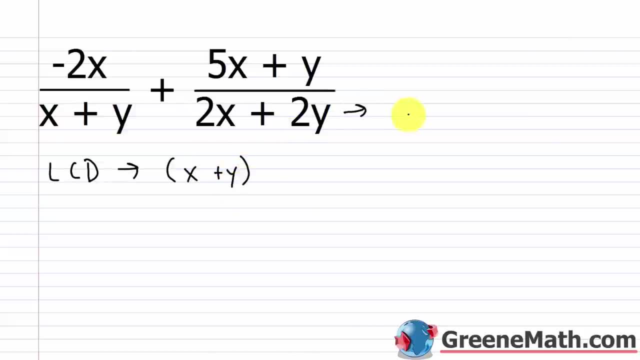 over here I can factor out a 2 so I could write this as 2 times the quantity x plus 1 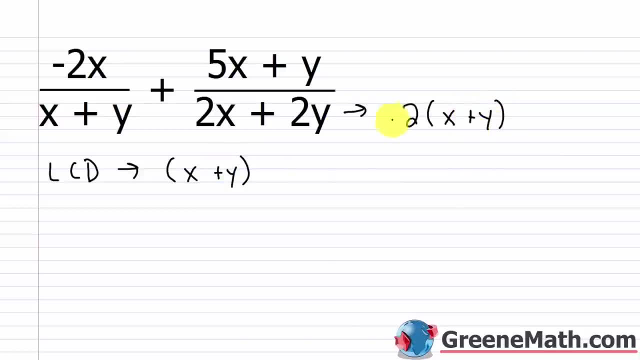 now I've already got an x plus y here I just need the 2 so the LCD is 2 times the quantity x plus y 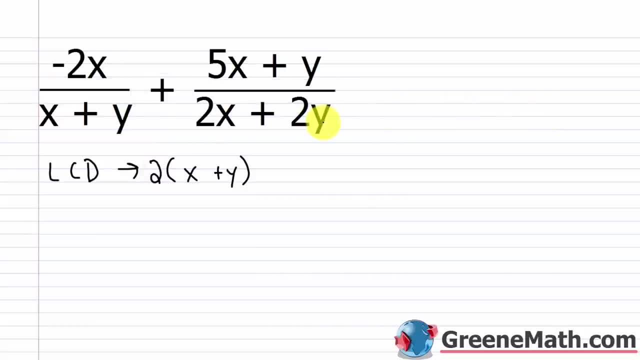 so because this denominator is already the LCD I don't need to change this rational expression 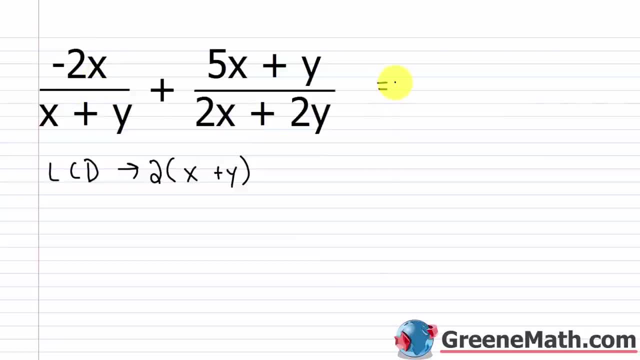 I just need to change the one on the left so what I'm going to do I'm going to multiply negative 2x over x plus y times what I'm missing 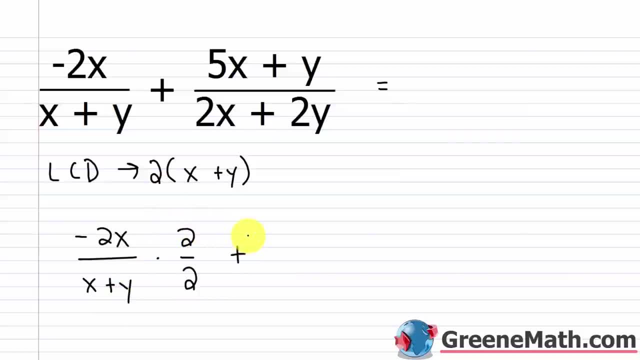 here is a 2 so 2 over 2 then I'm going to add to this the 5x plus y over 2 times the quantity x plus y ok so negative 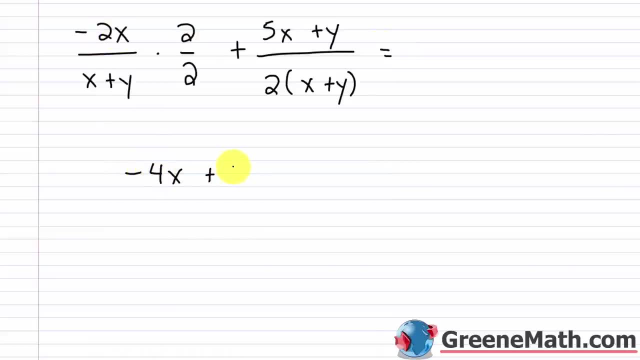 2x times 2 is negative 4x and then plus 5x plus y again over this common denominator of 2 times the quantity x plus y if I combine like terms here negative 4x plus 5x is x 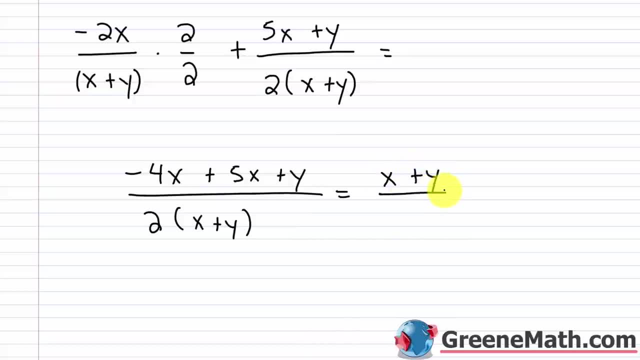 so what this gives me is x plus y in the numerator over 2 times the quantity x plus y in the denominator and so what I can see is I have a common factor of x plus y again to make this obvious go ahead and put this inside parentheses and put times 1 1 times anything is just itself so now I can cancel this factor with this factor right those are factors 2 is multiplying this so those two are factors 1 is multiplying this so again those two are factors so we cancel common 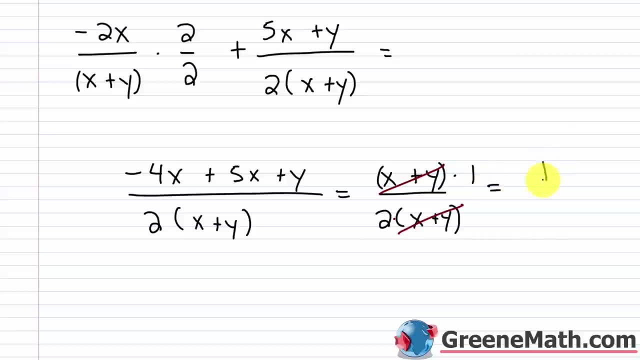 factors what I'm going to be left with is 1 over 2 or 1 half as my answer 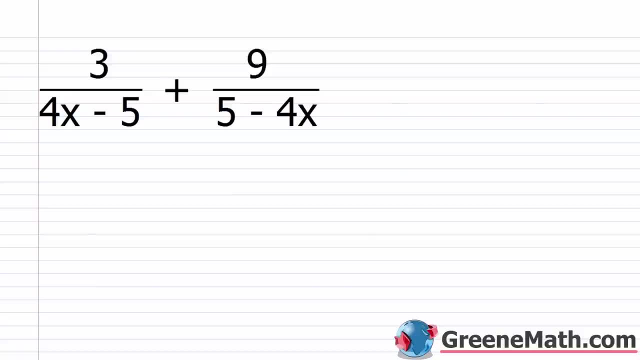 alright so let's look at one where the denominators are opposites so we have 3 over 4x minus 5 plus 9 over 5 minus 4x 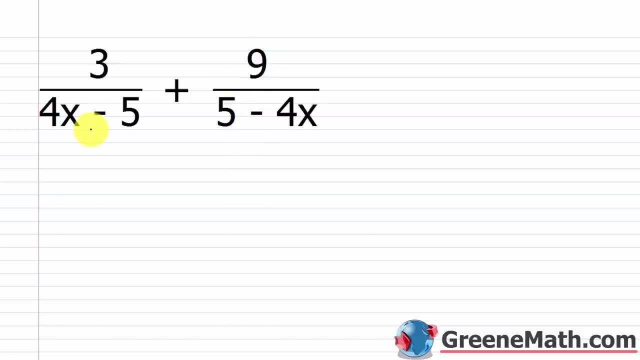 so remember we talked about this before if I see the same terms but they have different signs so in other words I could rearrange this and I could write this as negative 4x plus 5 if I want to so I have the same terms 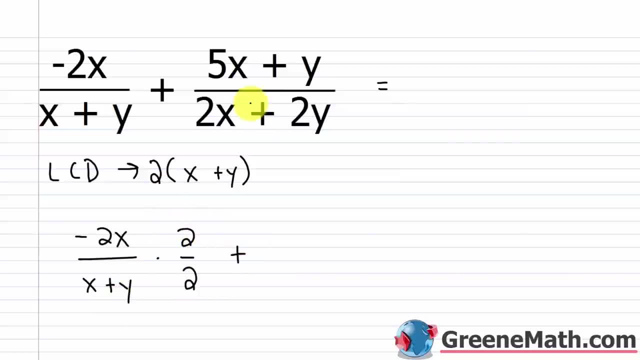 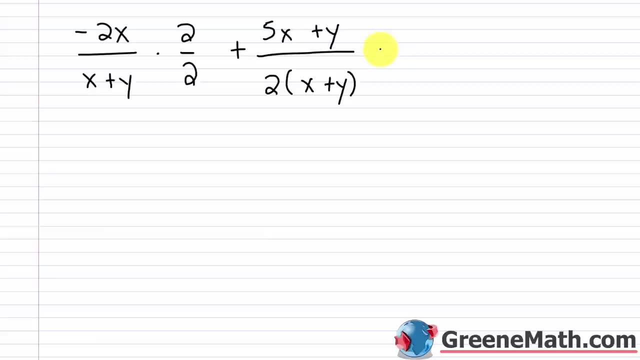 So 2 over 2.. Then I'm going to add to this the 5x plus y, over 2 times the quantity x plus y. Okay, So negative 2x times 2 is negative 4x, And then plus 5x plus y, again over this common denominator of 2 times the quantity x plus y. 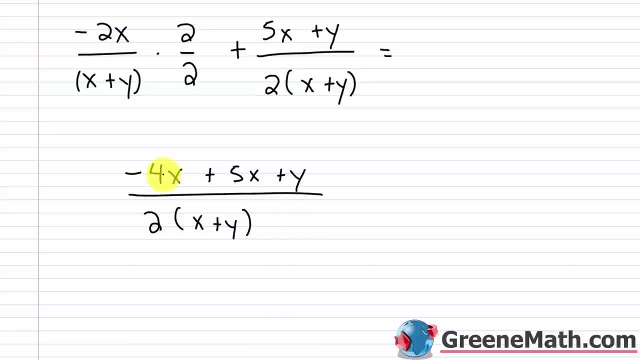 If I combine like terms here, negative 4x plus 5x is x. So what this gives me is x plus y in the numerator, over 2 times the quantity x plus y in the denominator, And so what I can see is I have a common factor of x plus y. 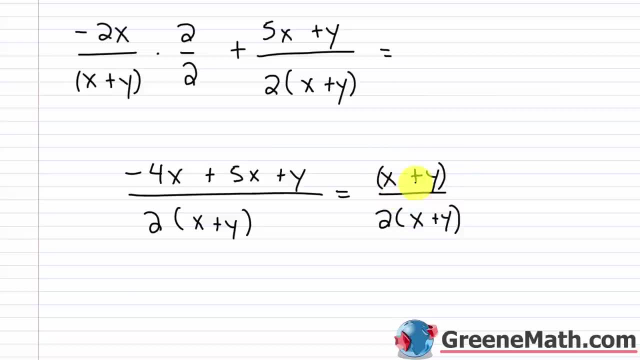 Again to make this obvious, go ahead and put this into the numerator, Put it inside parentheses and put times 1.. Right, 1 times, anything is just itself. So now I can cancel this factor with this factor Right, Those are factors. 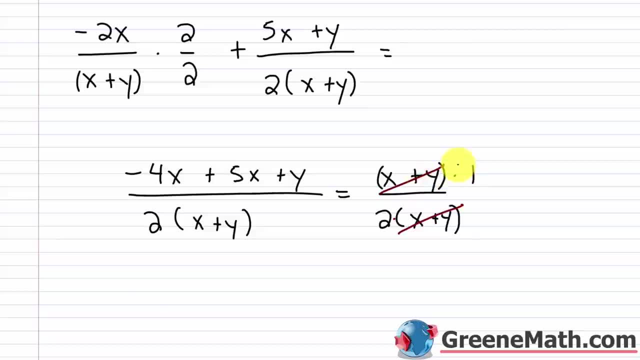 2 is multiplying this, So those two are factors. 1 is multiplying this, So again, those two are factors. So we cancel common factors. What I'm going to be left with is 1 over 2 or 1 half as my answer. 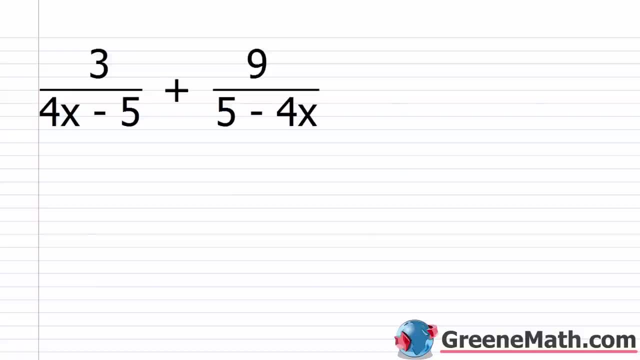 All right. So let's look at one where the denominators are opposites. We have 3 over 4x minus 5 plus 9 over 5 minus 4x. So remember we talked about this before. If I see the same terms, but they have different signs. 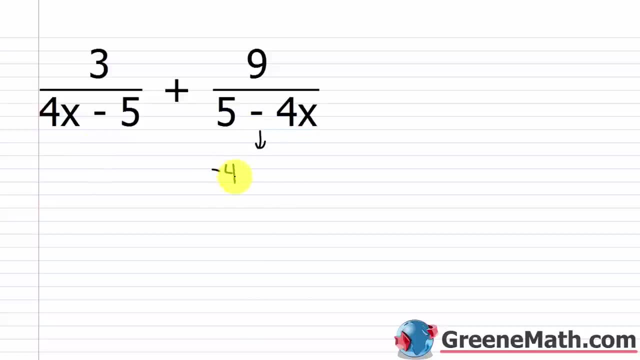 So, in other words, I could rearrange this and I could write this as negative 4x plus 5, if I want to. So I have the same terms, I have 4x and I have 4x, but the signs are different. 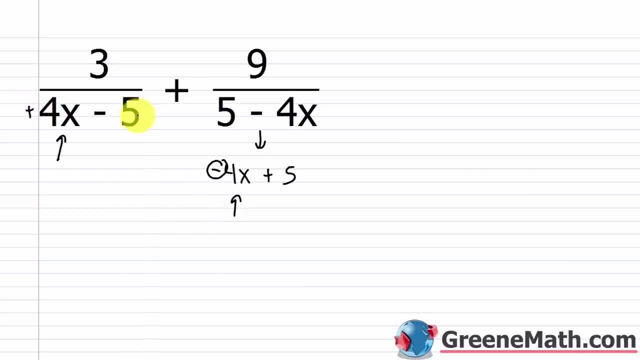 I have a negative and I have a positive, I have 5 and I have 5, but the signs are different. Right, I have a positive and I have a negative. Right, But same values, different signs, So those two are opposites. 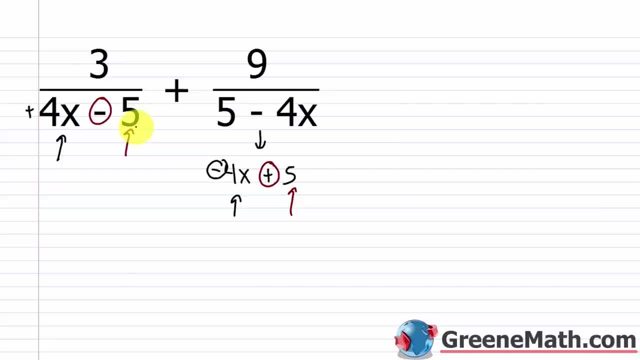 And to show that to you, just take one of them and factor out a negative 1.. So in other words, you put a negative 1 outside of parentheses and you change the sign of each term inside of the parentheses. So negative 4x would be 4x and then positive 5 would be negative 5.. 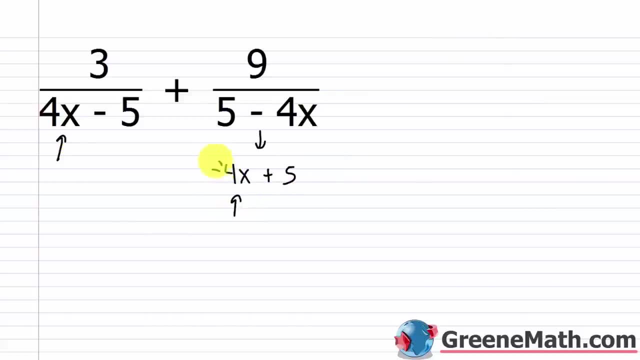 I have 4x and I have 4x but the signs are different I have a negative and I have a positive I have 5 and I have 5 but the signs are different I have a positive and I have a negative but same values different signs so those two are opposites and to show that to you just take one of them and factor out a negative 1 so in other words you put a negative 1 outside of parentheses and you change the sign of each term inside of the parentheses 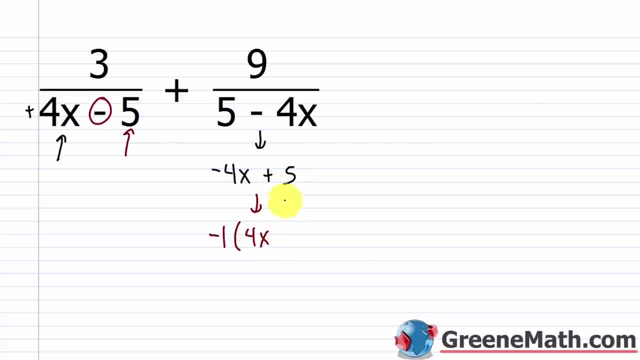 so negative 4x would be 4x and then positive 5 would be negative 5 now you can see that these two are the same with the difference of this being multiplied by negative 1 right so I have 4x minus 5 I have 4x minus 5 again this is being multiplied by negative 1 what can I do here 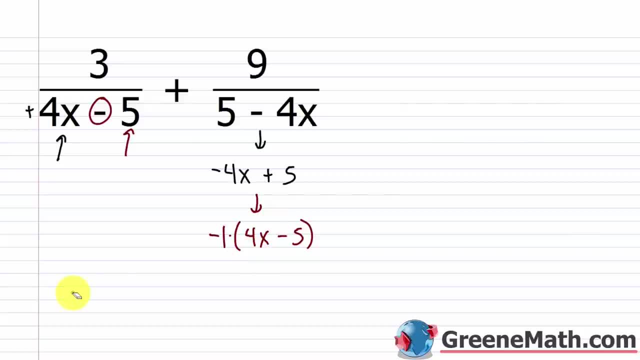 well I want you to recall that if I was working with the fractions let's say 5 over 7 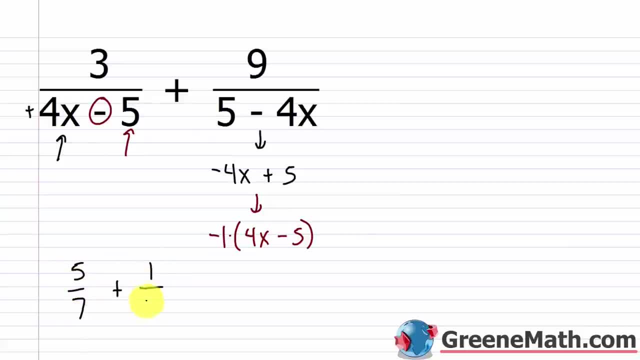 and I'm adding to this let's say 1 over negative 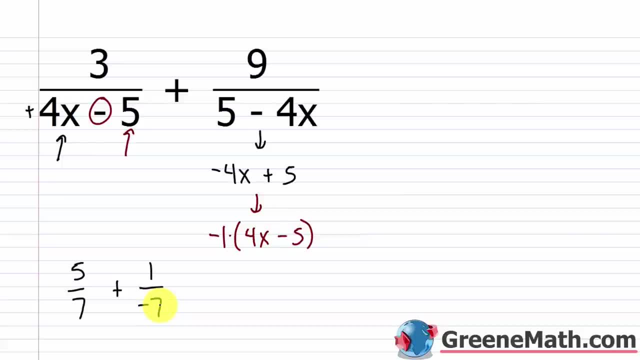 7 what could I do remember if the denominator is negative and the numerator is positive the fraction is negative so all I need to do is erase this put that here it's still the same value and I have that common denominator of 7 now 5 minus 1 is 4 over the common denominator of 7 it's the same thing here it's the same principle so really all I'm going to do I have the same denominator all I need to do is take this negative 1 move it into the numerator that's all I'm going to do 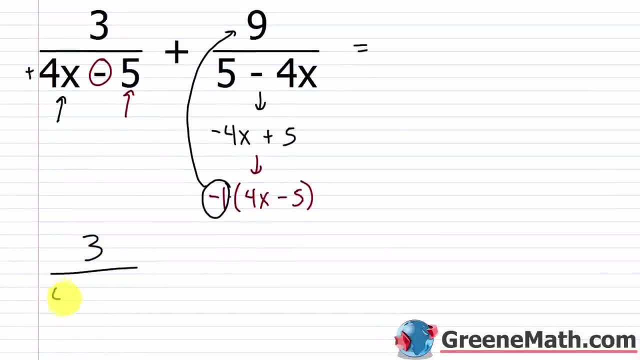 very very simple so I have 3 over 4x minus 5 and then plus I'm going to now make this negative 9 over 4x minus 5 ok all I did was move the negative from the denominator to the numerator again you can do that I just showed you that with regular fractions it's the same if negative 1 is multiplying this I can just move it up here and have the negative 1 multiply the 9 that's how I got negative 9 ok 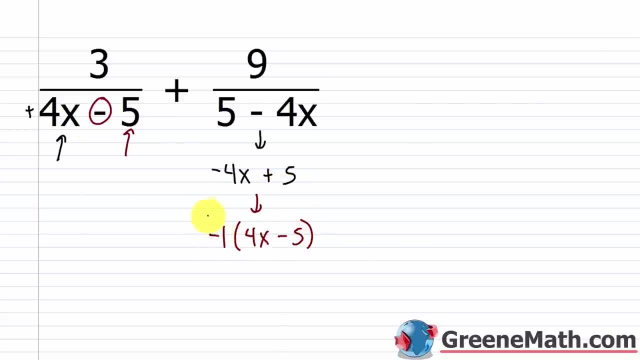 Now you can see that these two are the same, with the difference of this being multiplied by negative 5.. So I have 4x minus 5 and I have 4x minus 5.. Again, this is being multiplied by negative 1.. 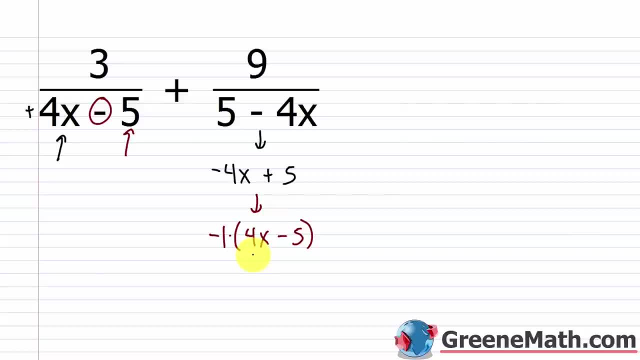 What can I do here? Well, I want you to recall that if I was working with the fractions, let's say 5 over 7, and I'm adding to this, let's say 1 over negative 7.. What could I do? 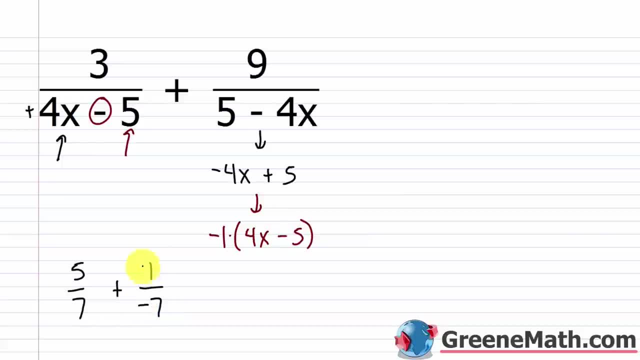 Remember, if the denominator is negative and the numerator is positive, the fraction is negative. So all I need to do is arrange this, Put that here, It's still the same value And I have that common denominator of 7.. Now, 5 minus 1 is 4 over the common denominator of 7.. 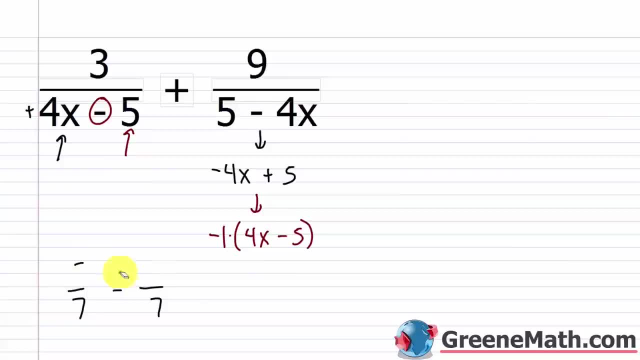 It's the same thing here. It's the same principle. So, really, all I'm going to do- I have the same denominator. All I need to do is take this negative 1, move it into the numerator And that's all I'm going to do. 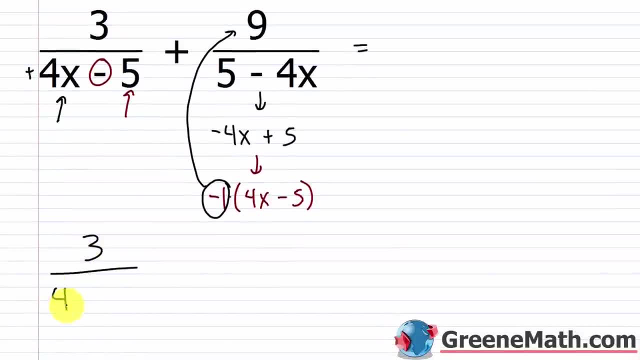 Very, very simple. So I have 3 over 4x minus 5.. And then plus. I'm going to now make this negative: 1.. Negative 9 over 4x minus 5.. All I did was move the negative from the denominator to the numerator. 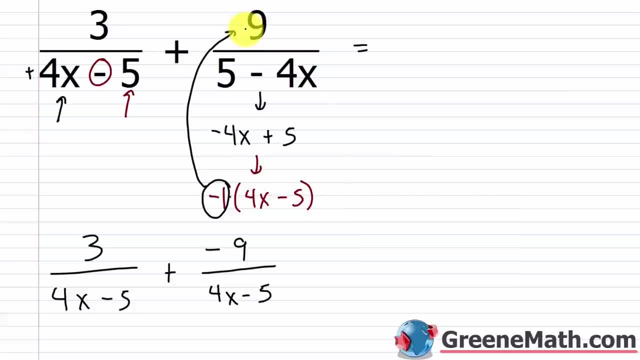 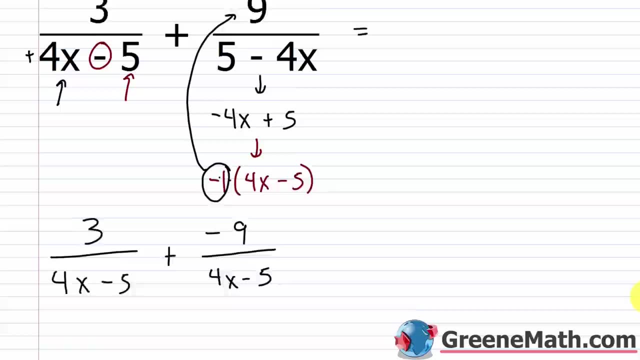 Again, you can do that. I just showed you that with regular fractions It's the same. If negative 1 is multiplying this, I can just move it up here and have the negative 1 multiply the 9.. That's how I got negative 9.. 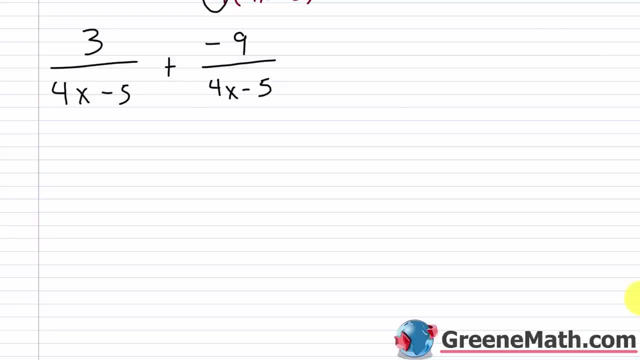 Okay, So now I have a common denominator And all I need to do is add 3 plus negative 9 is negative 6. What I get here is negative 6 over 4x minus 5. Very minimal work, And you can see there's nothing that I can do to cancel anything. 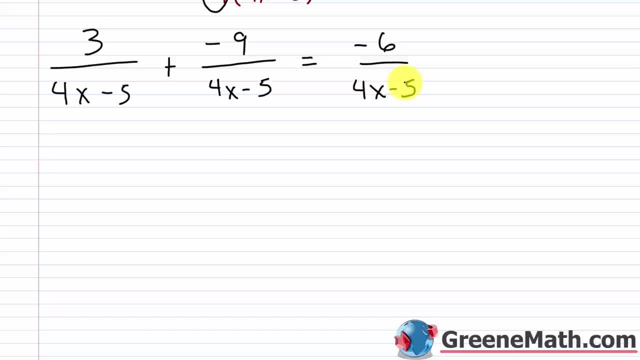 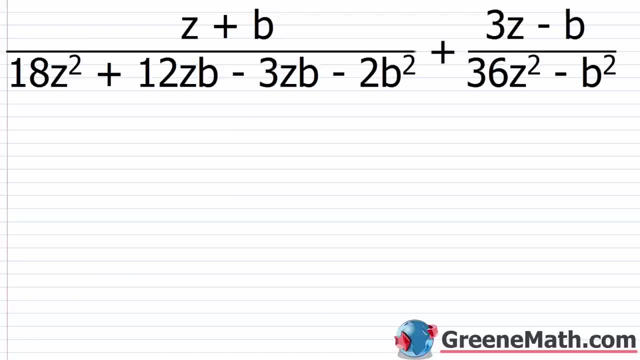 So that's my simplified answer. Again, negative: 6 over 4x minus 5.. All right, So we saved the best for last. Here's one that you might get Something extremely tedious. I have z plus b over 18z squared plus 12zb minus 3zb minus 2b squared plus 3z minus b. 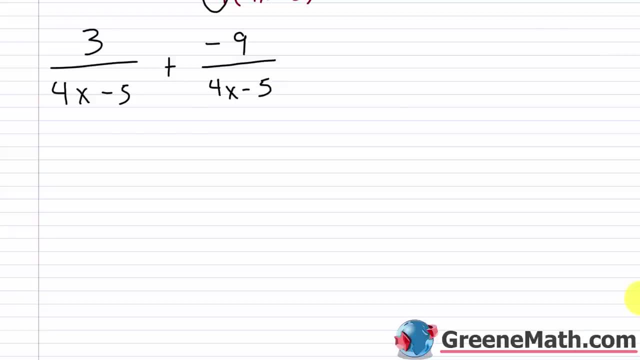 so now I have a common denominator and all I need to do is add 3 plus negative 9 is negative 6 so what I get here is negative 6 over 4x minus 5 very minimal work and you can see there's nothing that I can do to cancel anything so that's my simplified answer again negative 6 over 4x minus 5 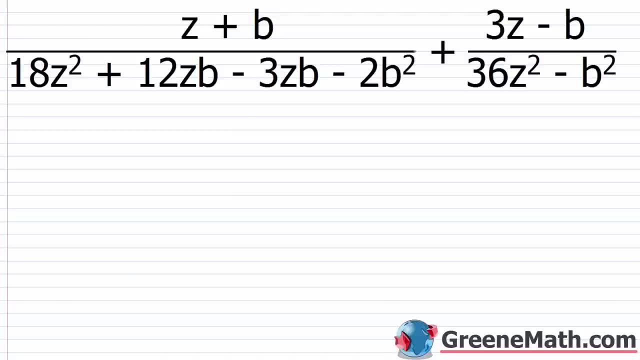 alright so we saved the best for last here's one that you might get something extremely tedious I have z plus b over 18z squared plus 12zb minus 3zb minus 2b squared 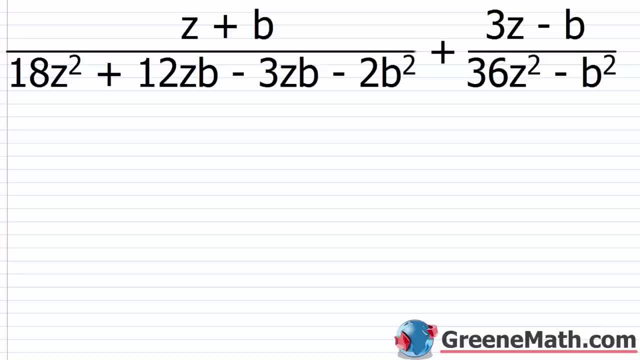 plus 3z minus b over 36zb z squared minus b squared 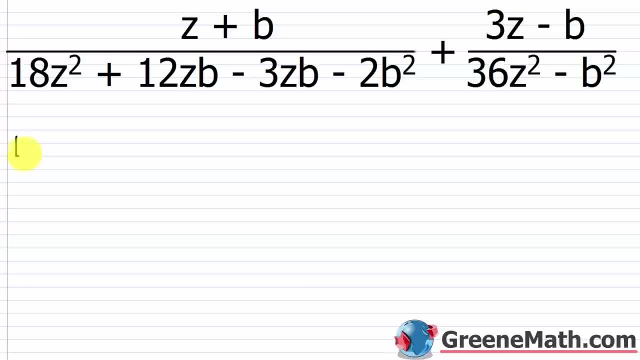 now to find the lcd I've got to factor these denominators first and this might take a little while now the first one I can factor by grouping it's a polynomial with 4 terms so let me just kind of do this here and we'll figure out our lcd in a minute 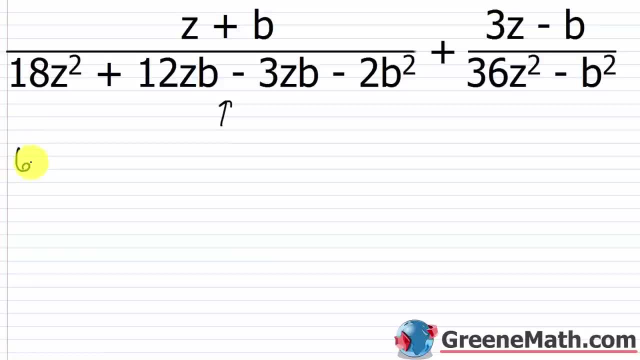 so I can pull out a 6z from the first group that would leave me with 3z plus 2b 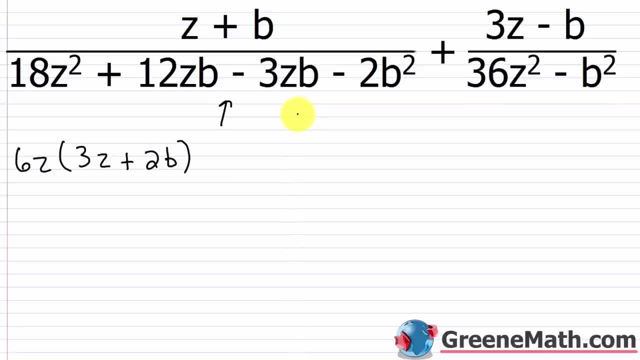 in the second group I can pull out a negative b negative b that would leave me with 3z plus 2b so I have a common binomial factor of 3z plus 2b and so this can be factored as 6z minus b times the quantity 3z 3z plus 2b ok let's erase this real quick 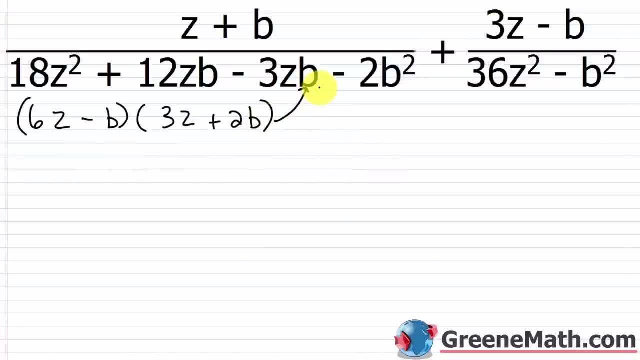 so we've got this as the factored form of that now when I look at 36z squared minus b squared what do you notice you've got 2 terms here and you've got a subtraction sign if you see that and you've got some squared things you might want to think about the difference of 2 squares again they're going to throw that at you all the time 36 is a perfect square it's 6 times 6 z squared is z times z b squared is b times b so really what this is this is 6z squared 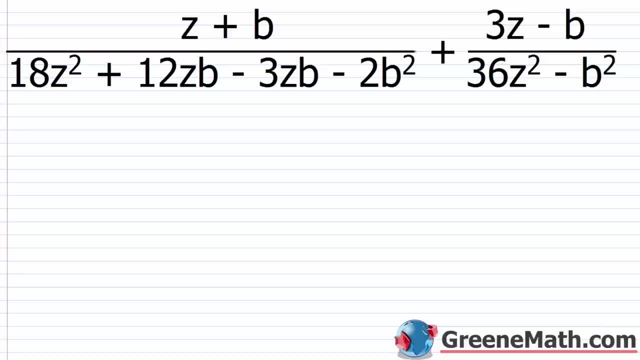 over 36.. z squared minus b squared. Now to find the LCD, I've got to factor these denominators first, And this might take a little while. Now, the first one I can factor by grouping It's a polynomial with four terms. 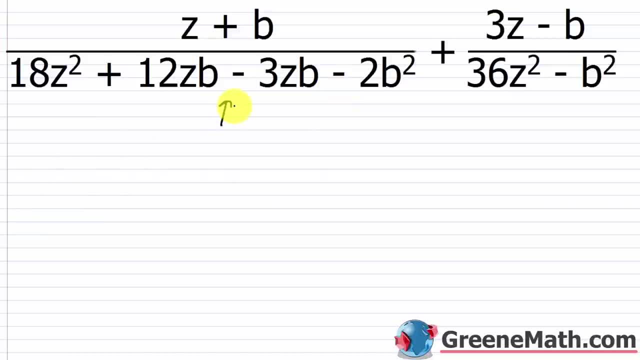 So let me just kind of do this here and we'll figure out an LCD in a minute. So I can pull out a 6z from the first group. That would leave me with 3z plus 2b. In the second group I can pull out a negative 3z. 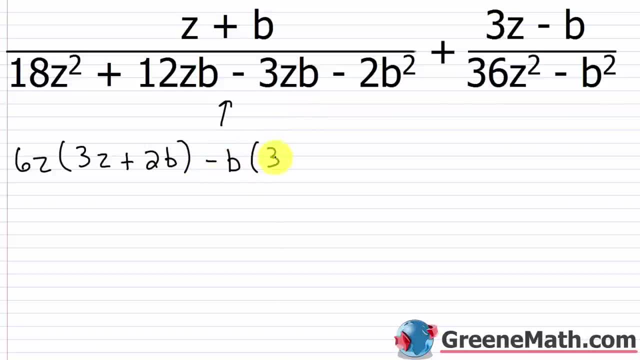 B, Negative b. That would leave me with 3z plus 2b. So I have a common binomial factor of 3z plus 2b, And so this can be factored as 6z minus b times the quantity 3z plus 2b. 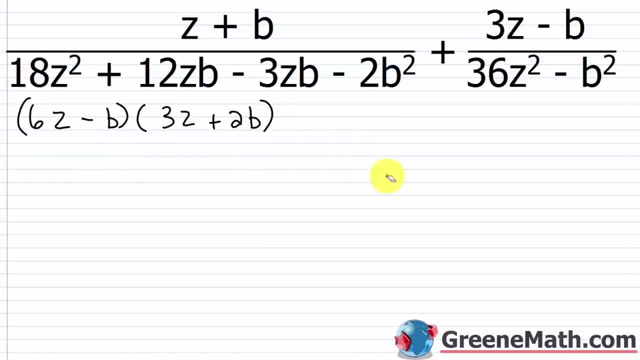 OK, So let's erase this real quick. So we've got this as the factored form of that. Now, when I look at 36z squared minus b squared, what do you notice? You've got two terms here and you've got a subtraction sign. 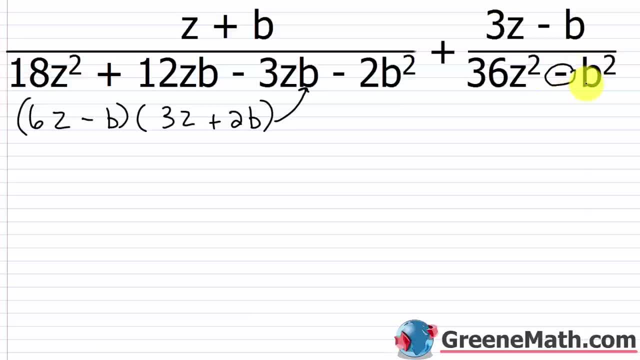 If you see that and you've got some squared things, you might want to think about the difference of two squares Again. they're going to throw that at you all the time. 36 is a perfect square. It's 6 times 6.. 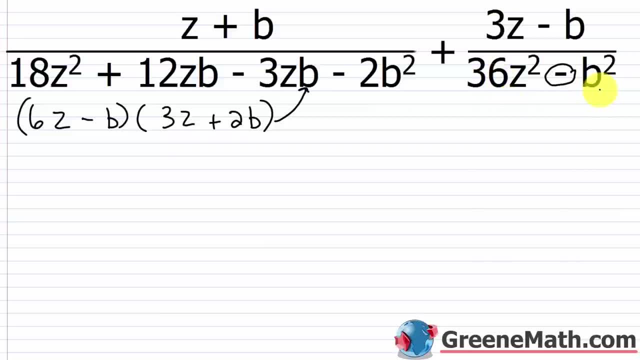 z squared is z times z. b squared is b times b. So really, what this is, this is 6z squared minus b squared, So this factors into 6z plus b times 6z minus b. Now what you can see is that you have this and this that are common. 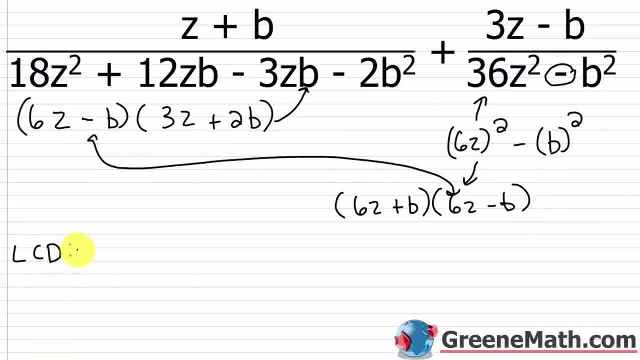 So when I build my LCD, what I'm going to have is one factor of 6z minus b- I don't need two- Then one factor of 6z plus b, Then one factor of 3z plus 2b. 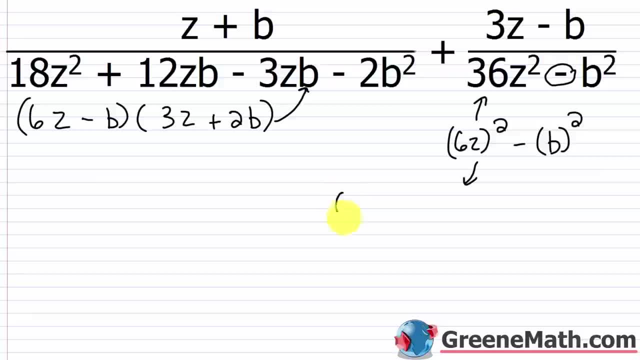 minus b squared and this factors into 6z plus b times 6z minus b now what you can see is that you have this and this that are common so when I build my LCD what I'm going to have is one factor of 6z minus b I don't need 2 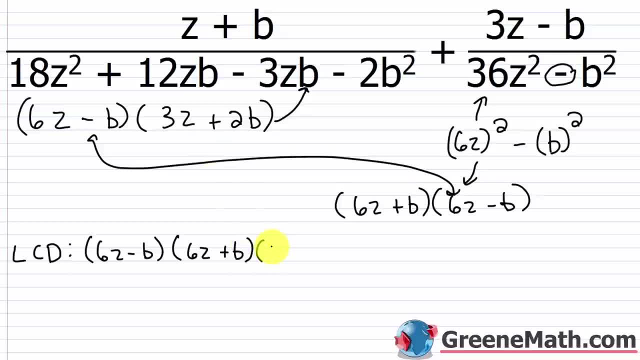 then one factor of 6z plus b then one factor of 3z plus 2b so that's my LCD 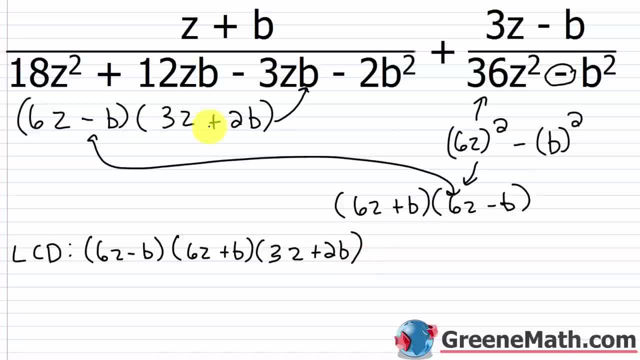 now what do I need over here over here I would be multiplying by just 6z plus b so I would have z plus b and this would be multiplied by again 6z plus b 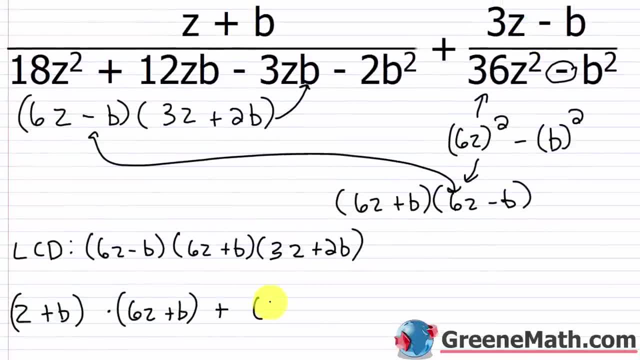 now for this one over here let me put plus I would have 3z minus b times what am I missing well I'm missing the 3z plus 2b 3z plus 2b 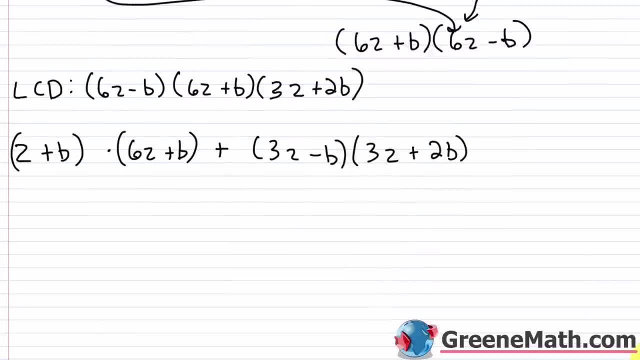 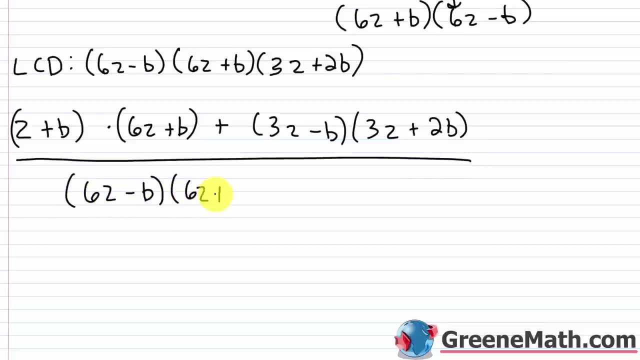 ok so let's go down here I know my LCD is this so let me write this over that so 6z minus b times 6z plus b times 3z plus 2b again just one that is pretty tedious 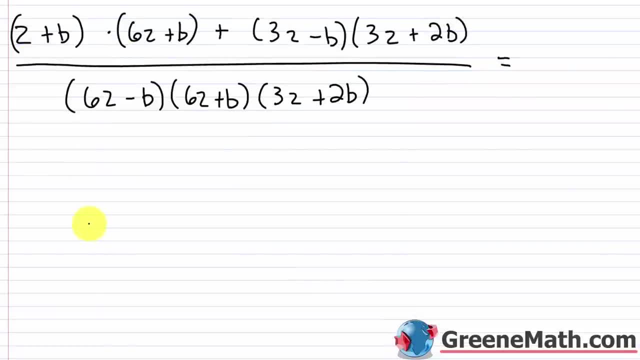 overall so I'm going to use FOIL 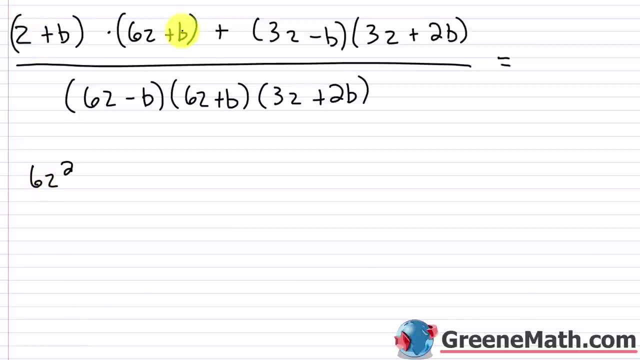 z times 6z is 6z squared z times b is zb zb b times 6z is plus 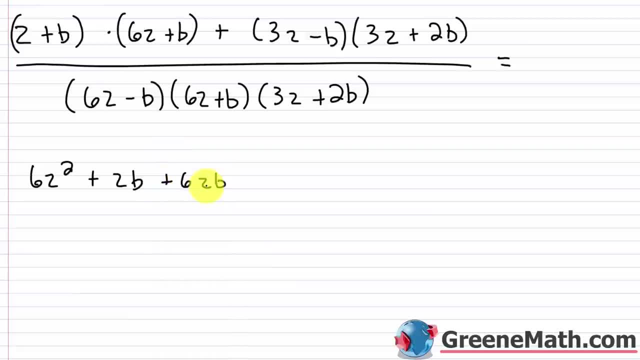 6zb if I combine these two I get plus 7zb so plus 7zb 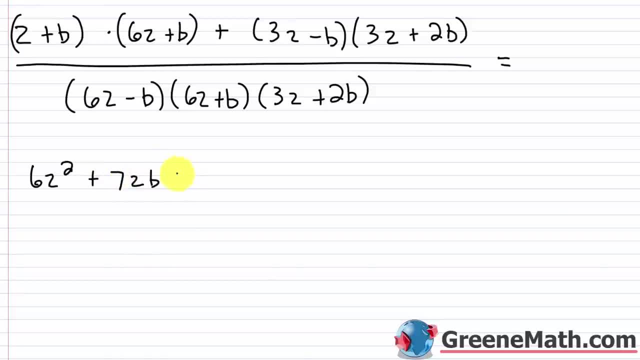 and then for the last b times b is b squared so plus b squared 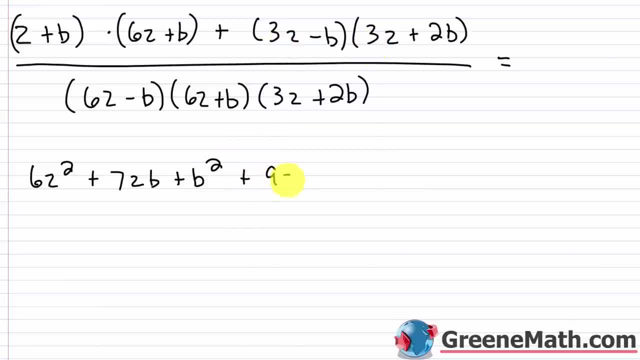 now over here 3z times 3z is 9z squared 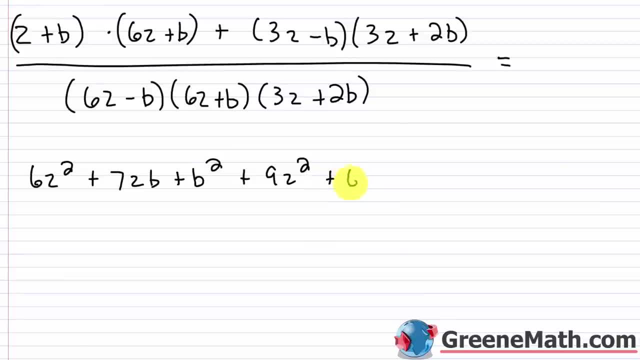 3z times 2b is plus 6zb negative b times 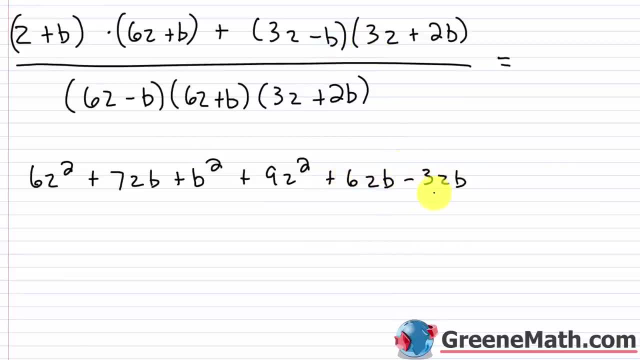 3z is minus 3zb if I combine like terms here I'd have plus 3zb 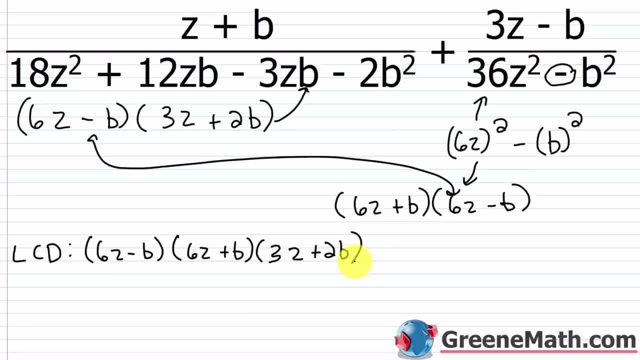 So that's my LCD. Now What do I need over here? Over here I would be multiplying by just 6z plus b, So I would have z plus b, and this would be multiplied by again 6z plus b. 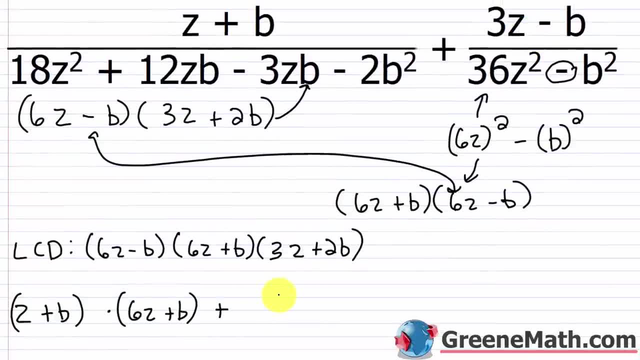 Now for this one over here. let me put plus, I would have 3z minus b times. what am I missing? Well, I'm missing the 3z plus 2b. 3z plus 2b, Okay. 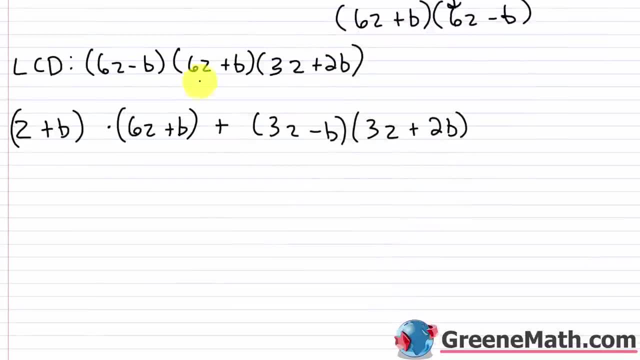 So let's go down here. I know my LCD is this, so let me write this over that. So 6z minus b times 6z plus b times 3z plus 2b- Again just one. that's pretty tedious overall. 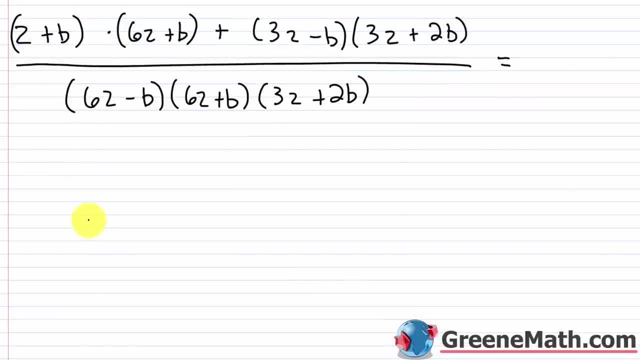 So I'm going to use FOIL: z times 6z is 6z squared z times b is zb, b times 6z is plus 6zb. If I combine these two I get plus 7zb, So plus 7zb. 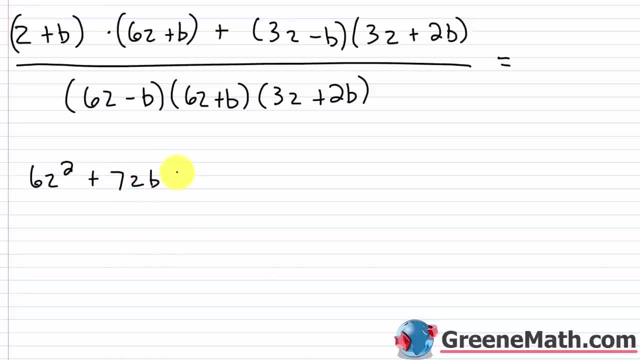 And then for the last, b times b is b squared, So plus b squared. Now over here: 3z times 3z is 9z squared. 3z times 2b is plus 6zb. Negative b times 3z is minus 3z squared. 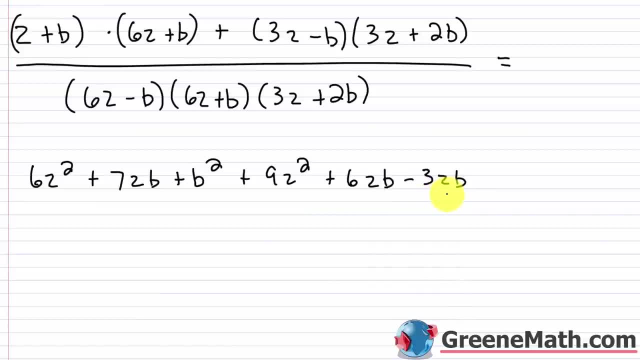 If I combine like terms here, I'd have plus 3zb Plus 3zb. And then, lastly, I have negative b times 2b, So minus 2b squared, And again all over that common denominator of 6z minus b times 6z, plus b times 3z plus 2b. 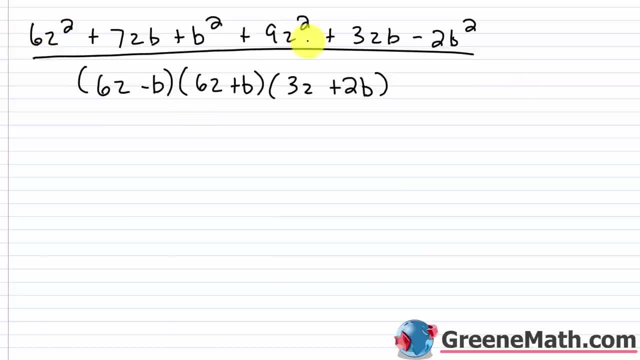 All right. So for like terms, I have 6z squared and 9z squared, That is 15z squared. I have 7zb and 3zb, That's 10zb. I have b squared and negative 2b squared. 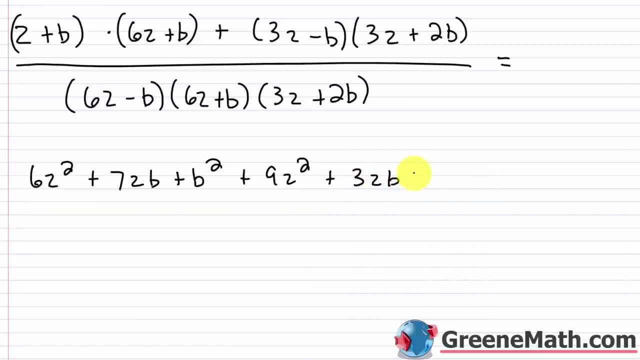 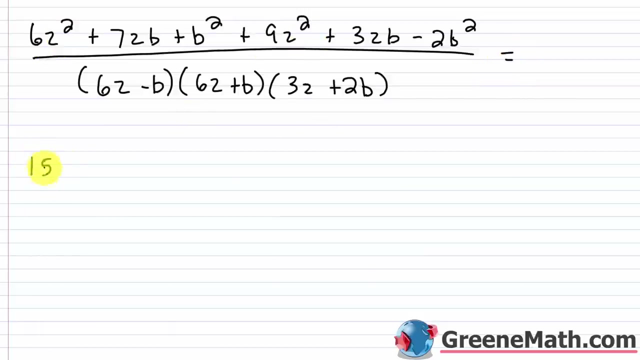 plus 3zb and then lastly I have negative b times 2b so minus 2b squared and again all over that common denominator of 6z minus b times 6z plus b times 3z plus 2b alright so for like terms I have 6z squared and 9z squared that is 15z squared I have 7zb and 3zb that's 10zb 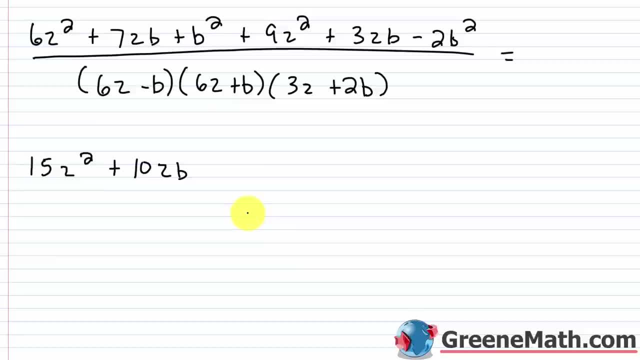 I have b squared and negative 2b squared so that's minus b squared 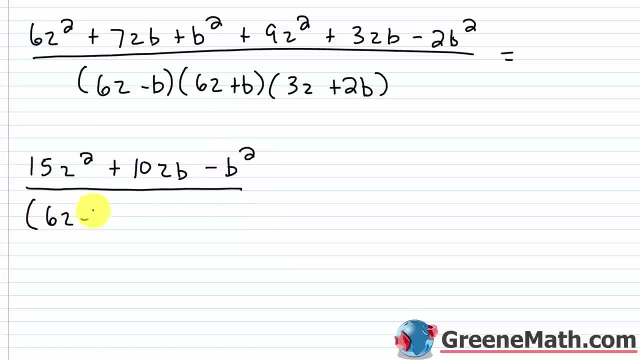 then this is all over again we have that 6z minus b times 6z plus b then times 3z plus 2b 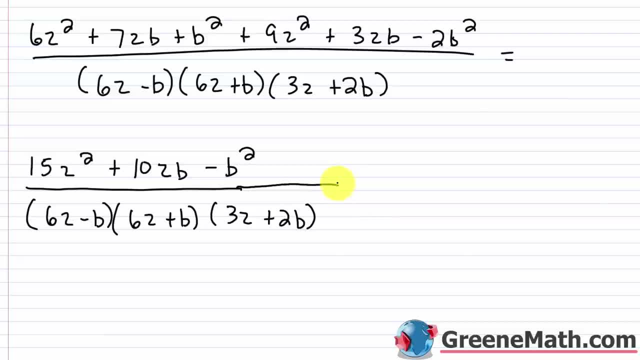 ok so one last step just to check to see if the numerator can be factored I need to find two terms now because we have two variables involved so I'm going to treat this last one like if it was a constant right remember this is usually 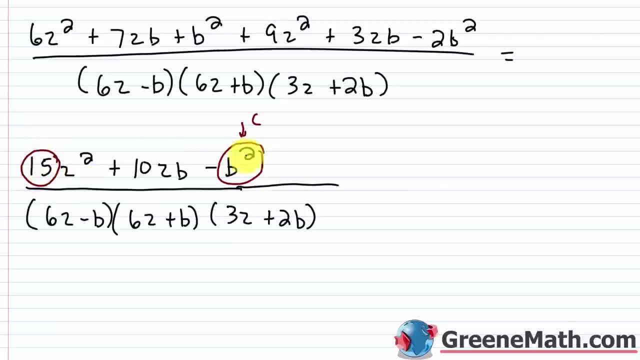 my c term so I'm going to say a the coefficient here times this guy right here so 15 times negative b squared is negative 15b squared so I need two terms that would multiply together to give me that and that would sum to give me 10b ok z is my squared variable here so I'm going to treat this b part right here as if it's part of that coefficient of z right so 10b 10b this is what I'm looking for for the sum 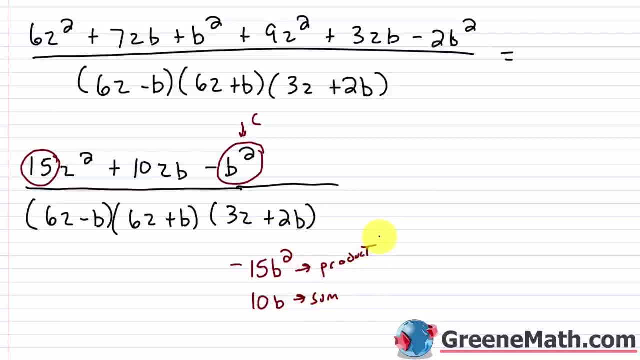 negative 15b squared for the product ok I know that's a little advanced we'll do a lot of that in algebra too but for right now just kind of follow me on this 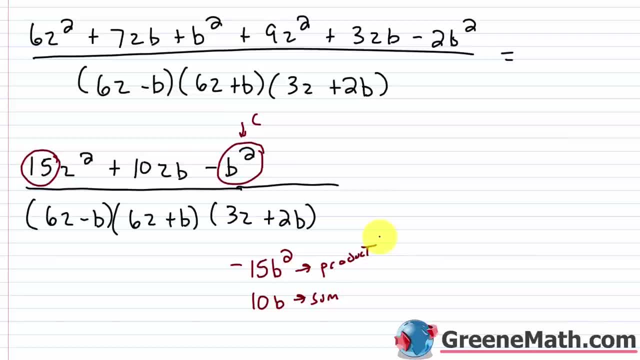 forget about the b part can you think of two integers that would multiply together to give you 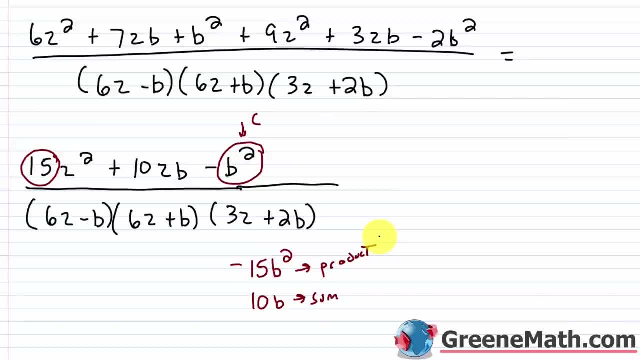 negative 15 and sum to give you 10 well you've got 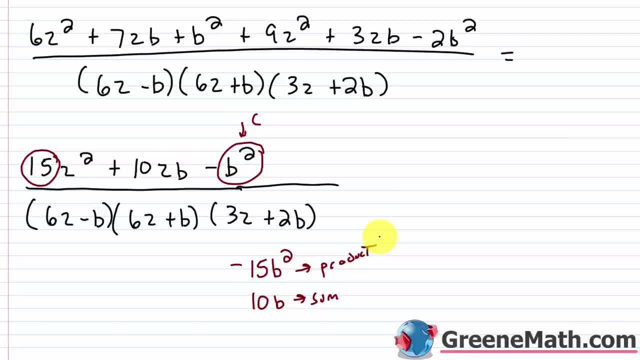 1 times 15 that's not going to work you can't change the signs around to give you that and you've got 3 times 5 so nothing you can really do with that so you can't get 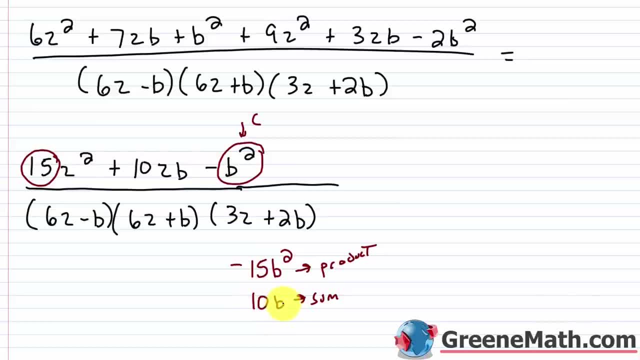 the number part to work out this part would work itself out automatically 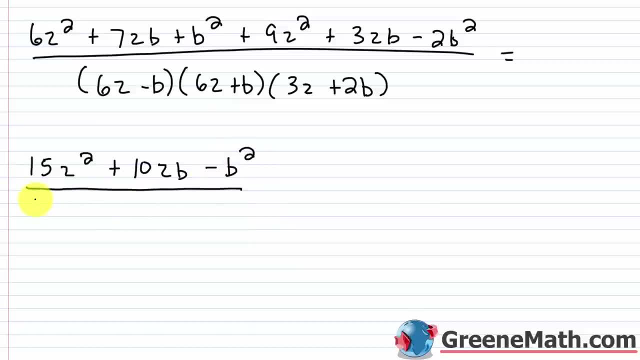 So that's minus b squared. Then this is all over Again. we have that 6z minus b, times 6z plus b, and then times 3z plus 2b. Okay, So one last step, just to check to see if the numerator can be factored. 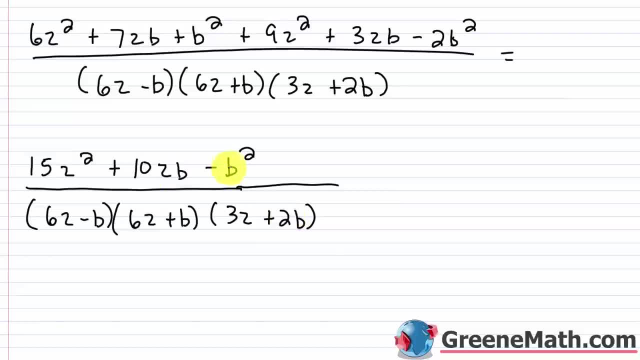 I need to find two terms now, Because we have two variables involved, So I'm going to treat this last one like if it was a constant. All right, Remember, this is usually my c term, So I'm going to say a. the coefficient here times this guy, right here. 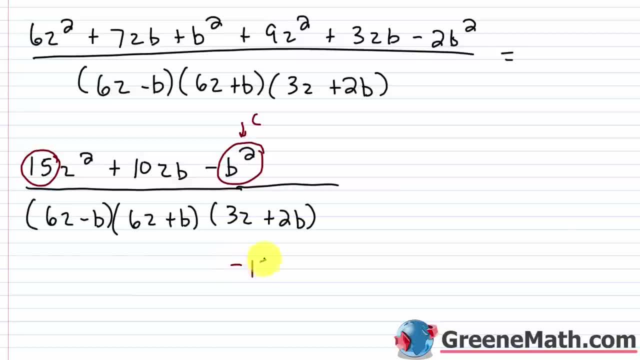 So 15 times negative b squared is negative 15b squared. So I need two terms that would multiply together to give me that And that would sum to give me 10b. Okay, z is my squared variable here, So I'm going to treat this b part right here. 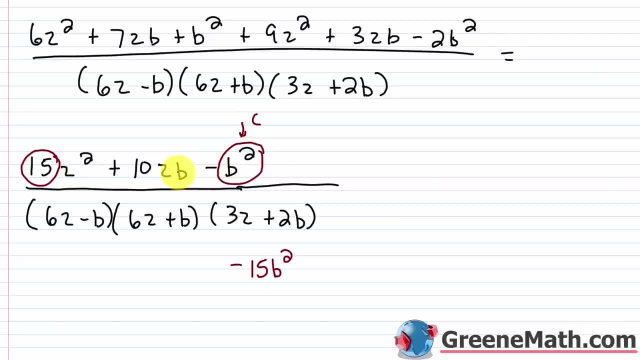 As if it's part of that coefficient of z Right. So 10b, 10b- This is what I'm looking for for the sum Negative, 15b squared for the product. Okay, I know that's a little advanced. 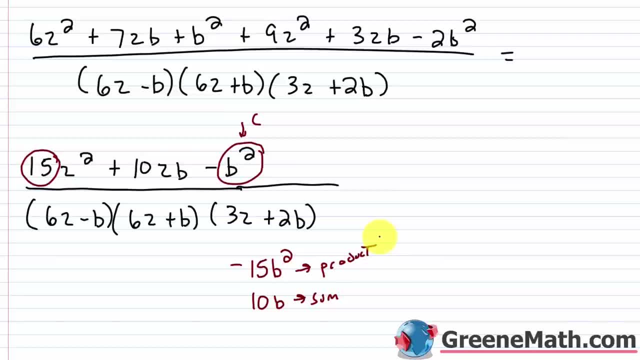 We'll do a lot of that in Algebra 2.. But for right now, just kind of follow me on this- Forget about the b part. Can you think of two integers that would multiply together to give you negative 15 and sum to give you 10?? 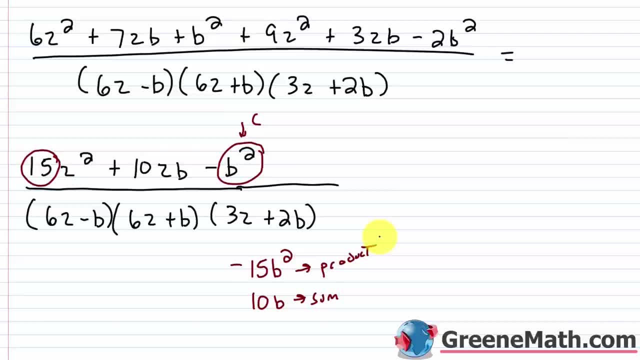 Well, you've got 1 times 15. That's not going to work. You can't change the signs around to give you that. And you've got 3 times 5. So nothing you can really do with that. So you can't get the number part to work out. 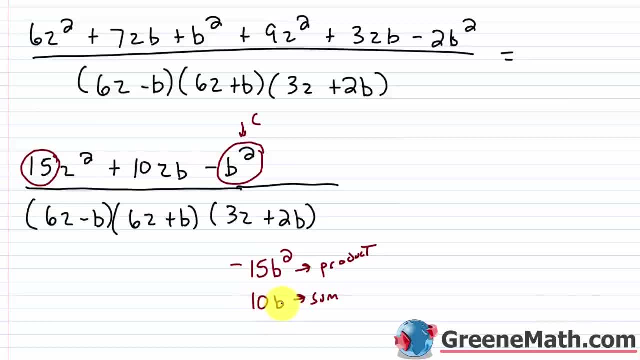 This part would work itself out automatically if you got the numbers to work out. So this is going to be a prime polynomial And we're not going to be able to factor it any further. So this is the simplified answer: 15z squared plus 10zb minus b squared. 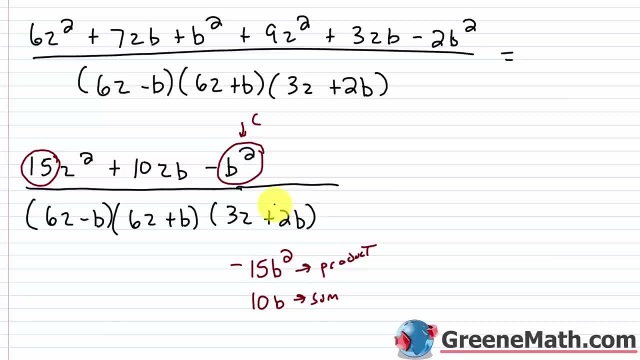 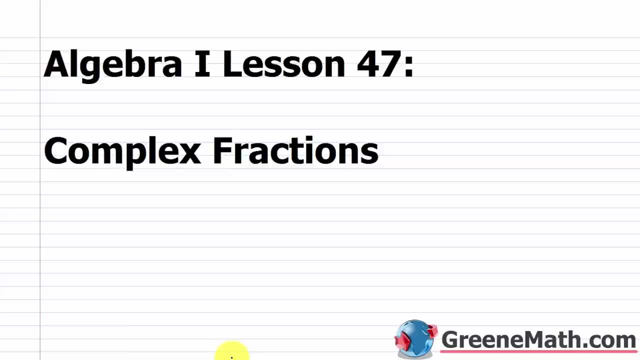 And this is over 6z minus b, times 6z plus b, and then times 3z plus 2b. Hello, This is Algebra 1, Lesson 47.. In this video we're going to learn about complex fractions. So I know not all of you took my course on pre-algebra. 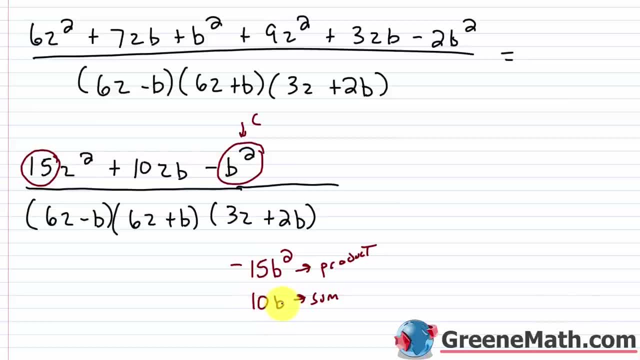 if you've got the numbers to work out so this is going to be a prime polynomial and we're not going to be able to factor it any further so this is the simplified answer 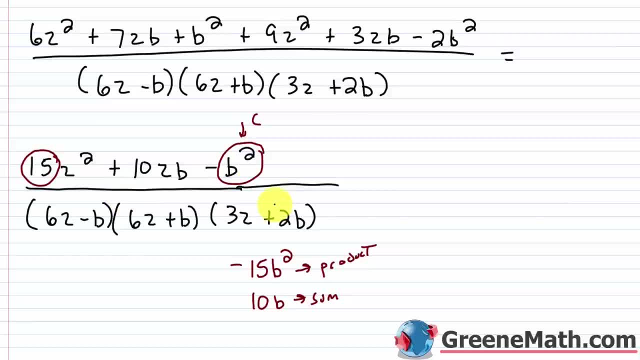 15z squared plus 10zb minus b squared and this is over 6z minus b 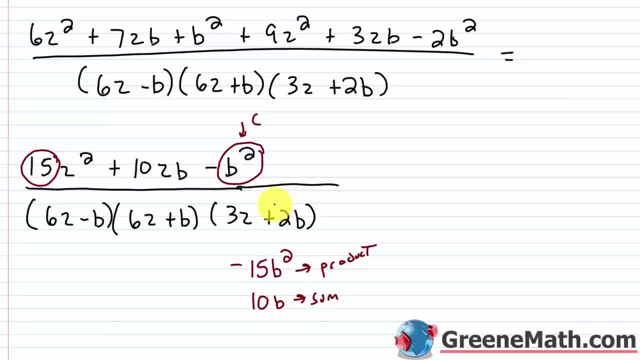 times 6z plus b and then times 3z plus 2b 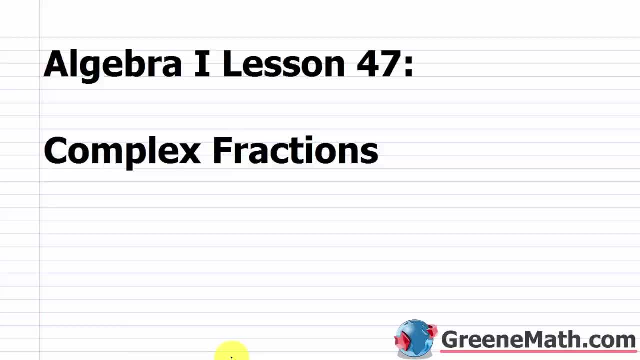 hello and welcome to algebra 1 lesson 47 in this video we're going to learn about complex fractions so i know not all of you took my course on 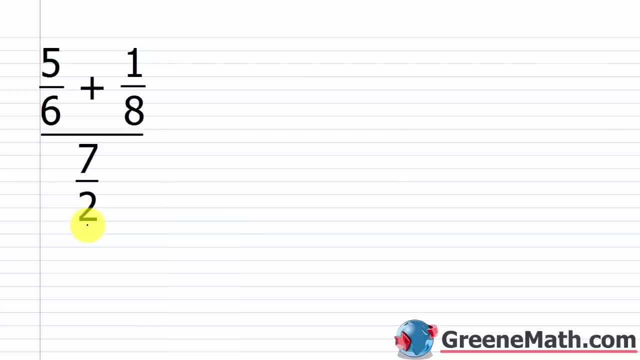 pre-algebra but hopefully before you got into the algebra 1 course you're currently in you've at least seen complex fractions at some point now what is a complex fraction let's just start out with that well it's a fraction that has a fraction in its numerator its denominator or both the numerator and the denominator so for example here we have 5 6 plus 1 8th over 7 halves so there is a fraction there's actually two fractions being added together in this case in the numerator 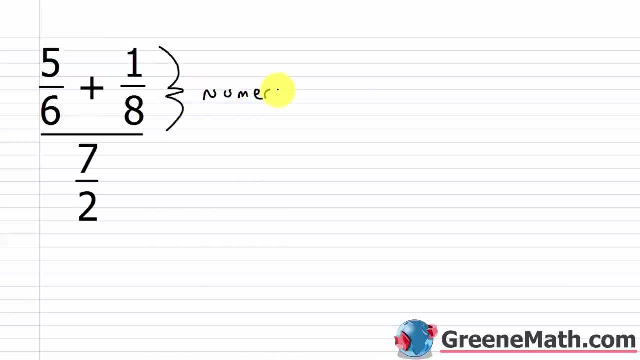 of the complex fraction this is the numerator 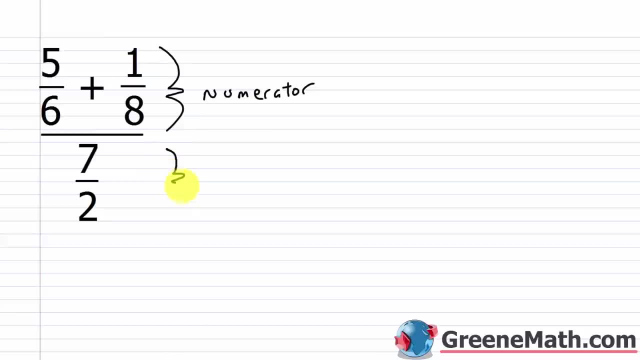 and there's also a fraction in the denominator you have 7 halves there 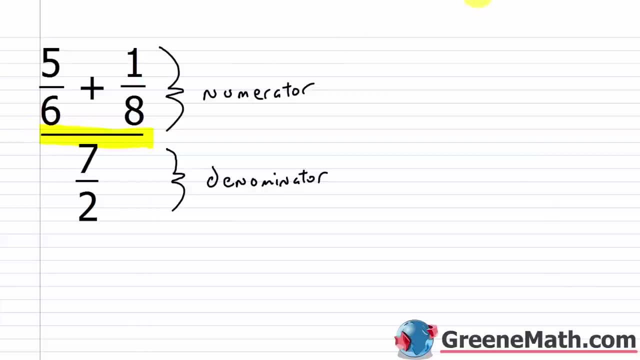 and then you can kind of think about this as your main division or your main fraction bar so your main division 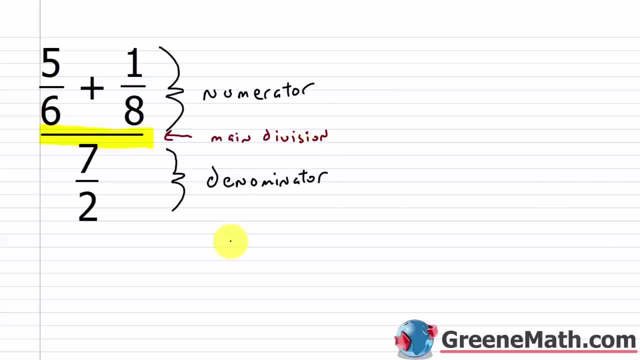 and why do i say main division remember if you have fractions you're dividing the numerator by the denominator something like 9 over 3 is the same as 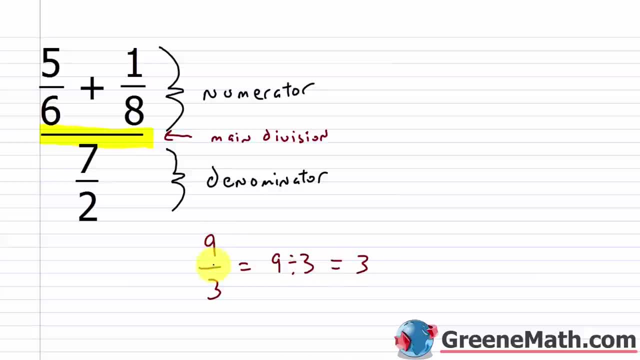 9 divided by 3 which is 3 right it's the numerator divided by 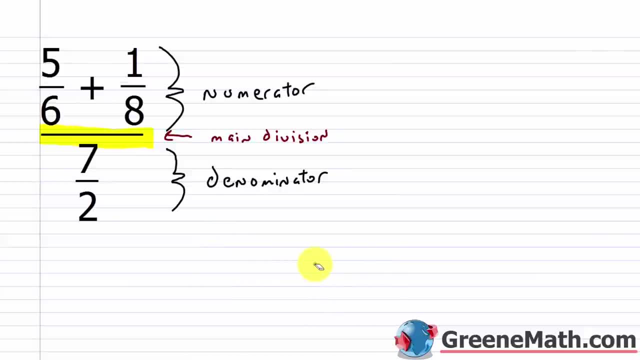 the denominator it is no different here with a complex fraction we have this numerator here although it's a complex numerator 5 6 plus 1 8th 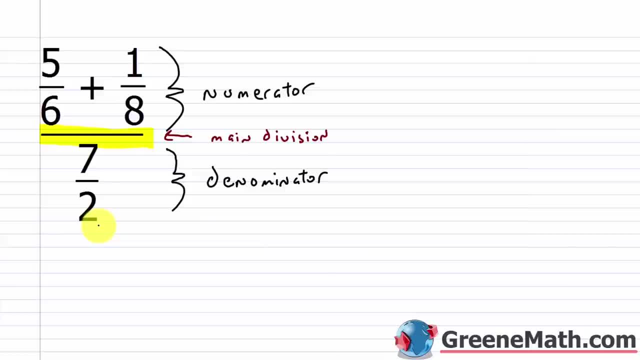 is divided by this denominator here 7 halves 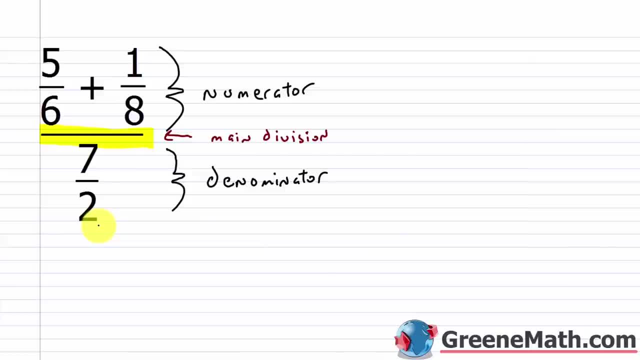 so how do we go about simplifying one of these well i gave you two methods in my pre-algebra course to do so the first one and one that we probably use most often is to simplify the numerator and 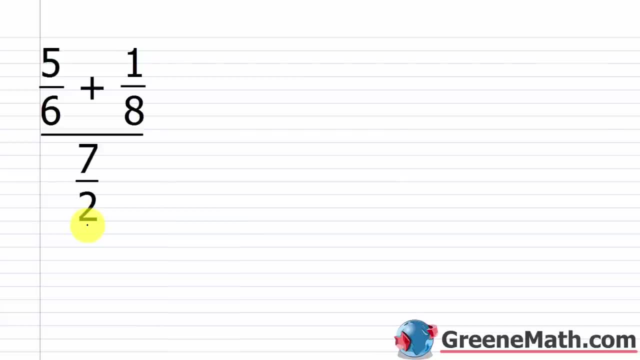 But hopefully, before you got into the Algebra 1 course you're currently in, you've at least seen complex fractions at some point. Now, what is a complex fraction? Let's just start out with that. Well, it's a fraction that has a fraction in its numerator, its denominator, or both the numerator and the denominator. 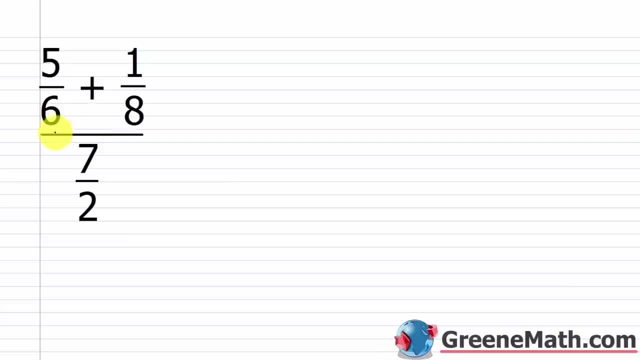 So, for example, here We have 5 sixths plus 1 eighths, over 7 halves. So there is a fraction. There's actually two fractions being added together, in this case in the numerator of the complex fraction. This is the numerator: 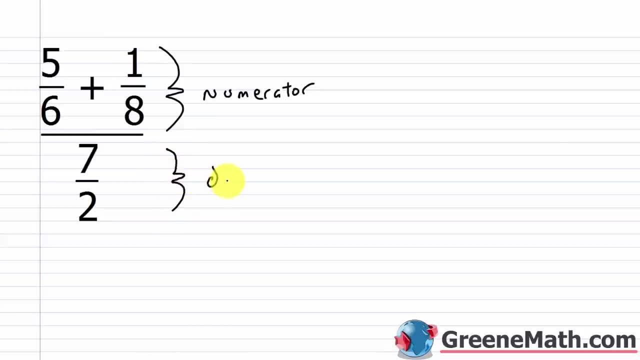 And there's also a fraction in the denominator. You have 7 halves there And then you can kind of think about this as your main division or your main fraction bar. So your main division. And why do I say main division? Remember, if you have fractions you're dividing the numerator by the denominator. 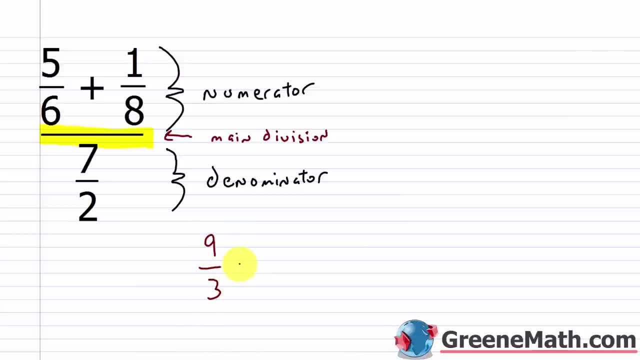 Something like 9 over 3 is the same as 9 divided by 3, which is 3.. It's the numerator divided by the denominator. It is no different here with a complex fraction. We have this numerator here, Although it's a complex numerator. 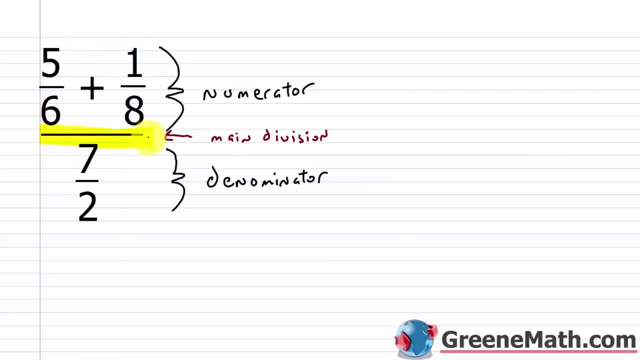 5 sixths plus 1 eighths is divided by this denominator, here 7 halves. So how do we go about simplifying one of these? Well, I gave you two methods in my pre-algebra course to do so. The first one, and one that we probably use most often, is to simplify the numerator and denominator separately. 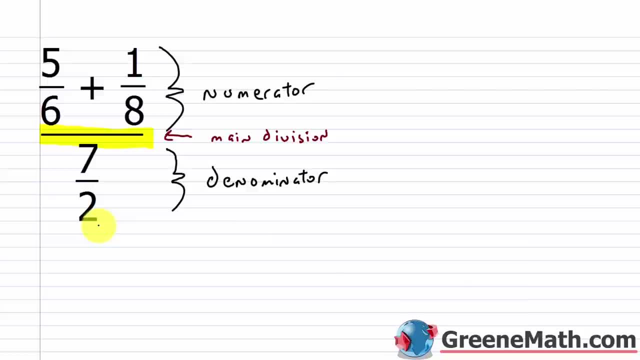 Then you would just perform the main division. So, for example, if I wanted to start out, if I had 5 sixths plus 1 eighths- Let's just deal with this part first- I would get a common denominator going. 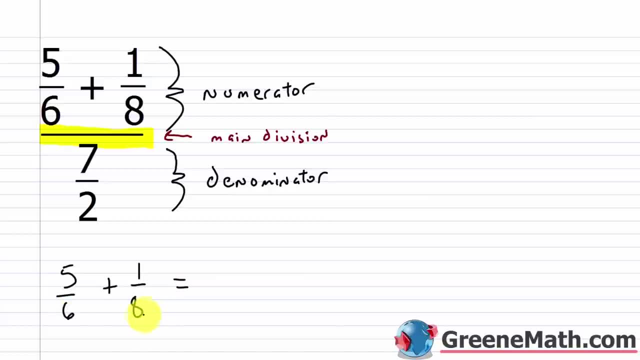 And for this one, 6 factors into 3 times 2.. 8 factors into 2 times 2 times 2.. So the LCD would be 2 times 2 times 2 times 3.. Right, which is what? 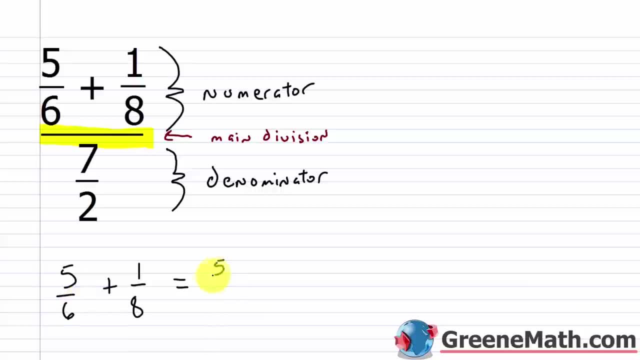 It's 8 times 3 or 24.. So I would take 5 sixths and I would multiply by 4 over 4.. And then I would take 1 eighths and I would multiply by 3 over 3.. 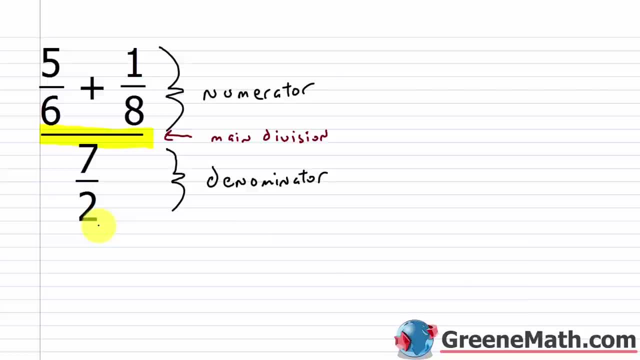 denominator separately then you would just perform the main division so for example if i wanted to start out if i had 5 6 plus 1 8th let's just deal with this part first i would get a common denominator going and for this one 6 factors into 3 times 2 8 factors into 2 times 2 times 2 so the lcd would be 2 times 2 times 2 times 3 right which is what it's 8 times 3 or 24 so i would take 5 6 and i would multiply by 4 over 4 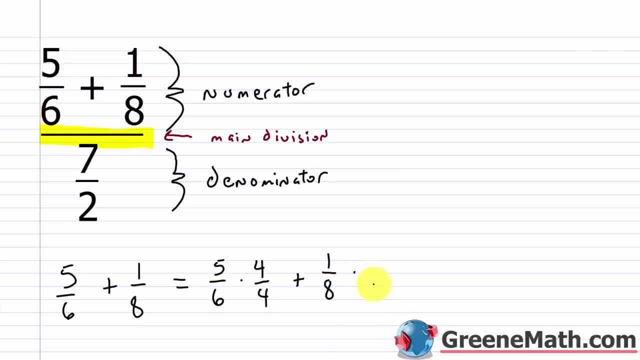 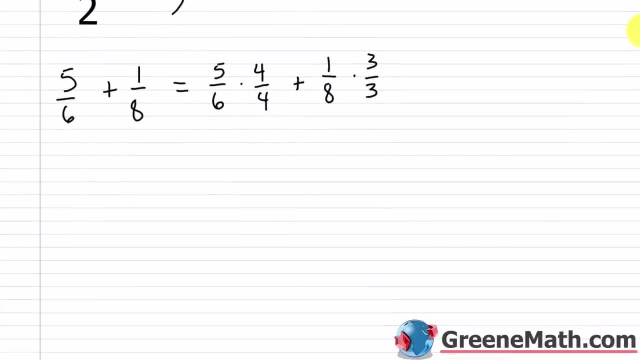 and then i would take 1 8th and i would multiply by 3 over 3 let me scroll down i'm going to take this off the screen for a minute but we'll come back to it so 5 times 4 is 20 plus 1 times 3 is 3 and this is over that common denominator of 24 so 20 plus 3 is 23 and then over 24 so if i simplify the numerator of the complex fraction i would get 23 over 24 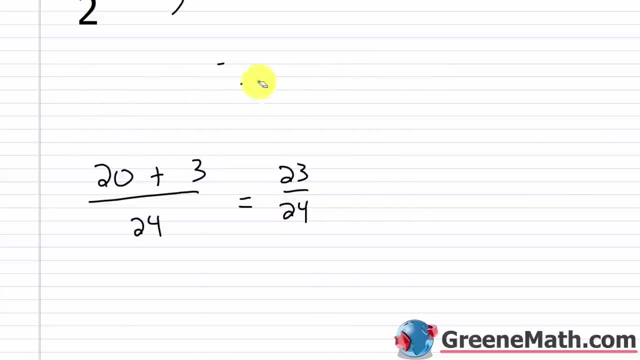 so let's just erase all this and go back up to the top 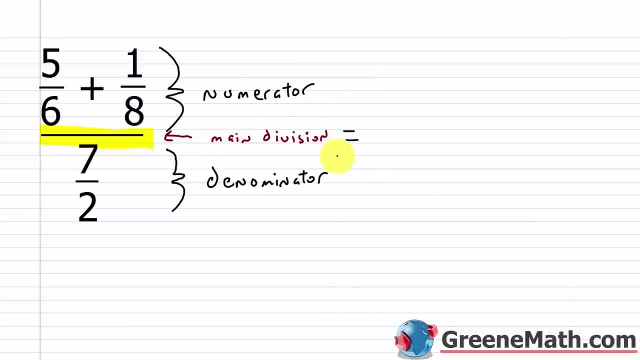 so i'm going to put equals out here i know i wrote a bunch of stuff but essentially what i'm doing is i'm saying the numerator of the 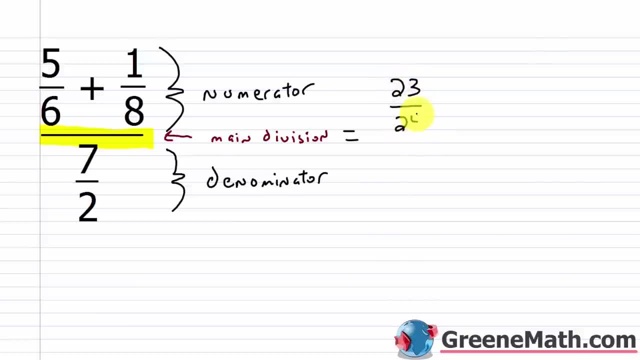 complex fraction is 23 over 24 then the denominator of the complex fraction is 7 halves so we think about it as 23 over 24 divided by 7 halves and if it makes you feel more comfortable you can write it like this this is 23 over 24 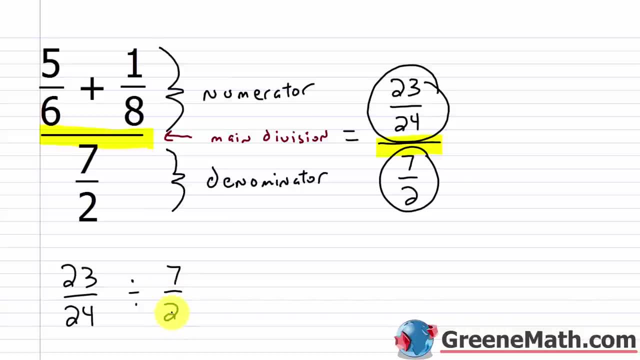 divided by 7 halves we all know how to divide with fractions we take the first fraction or the left most fraction in this case you think about that as the top fraction and we multiply by the reciprocal of the fraction on the right or the second fraction so this would be 23 over 24 times flip this guy 2 over 7 in this case you take again 23 over 24 times take the reciprocal of the fraction 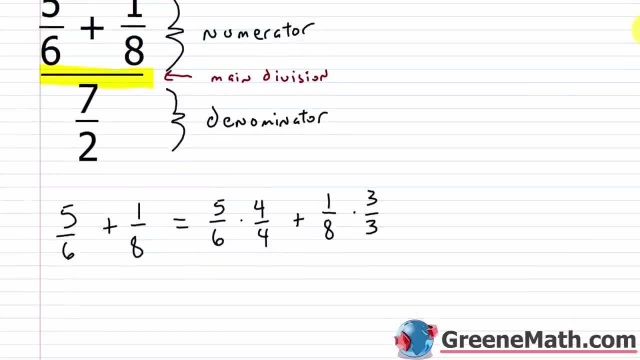 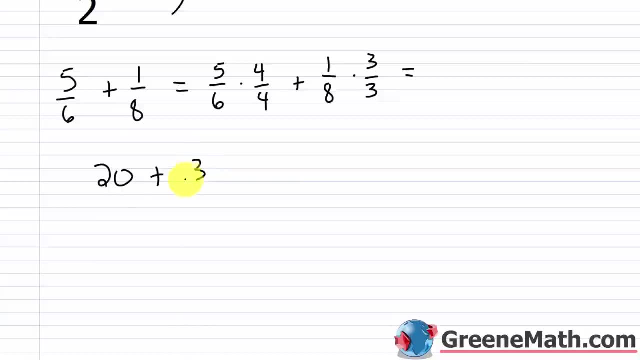 Let me scroll down. I'm going to take this off the screen for a minute, but we'll come back to it. So 5 times 4 is 20.. Plus 1 times 3 is 3.. And this is over that common denominator of 24.. 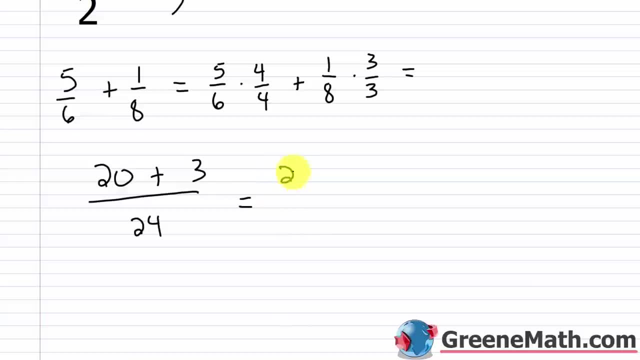 So 20 plus 3 is 23. And then over 24.. So if I simplify the numerator of the complex fraction, I would get 23 over 24.. So let's just erase all this And go back up to the top. 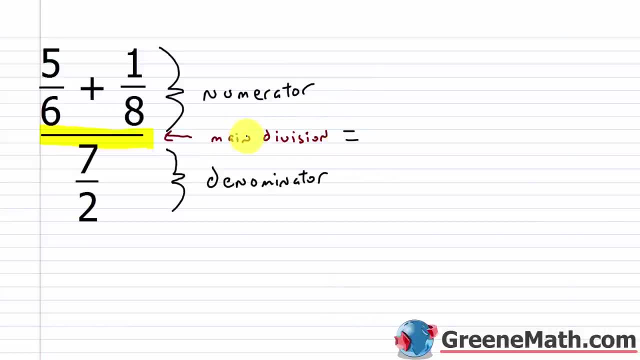 So I'm going to put equals out here. I know I wrote a bunch of stuff, but essentially what I'm doing is I'm saying the numerator of the complex fraction is 23 over 24.. Then the denominator of the complex fraction is 7 halves. 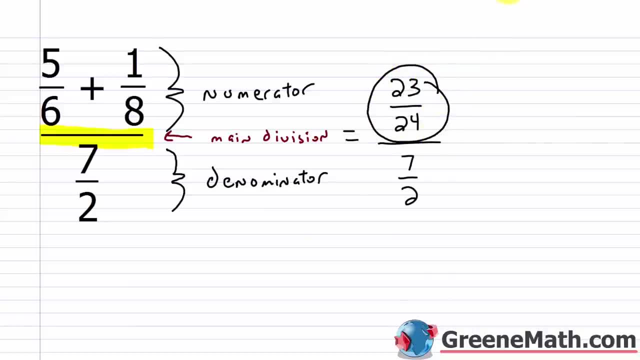 So we think about it as 23 over 24, divided by 7 halves, And if it makes you feel more comfortable, you can write it like this. You can say: okay, well, this is 23 over 24, divided by 7 halves. 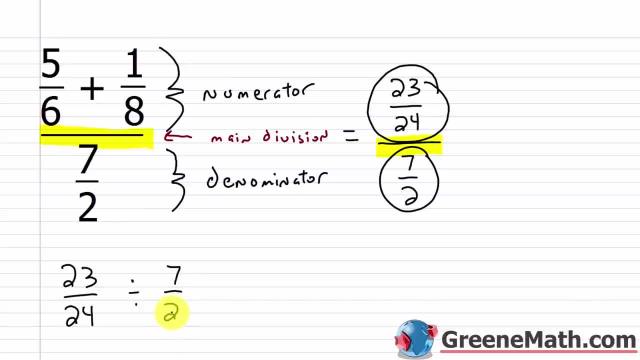 We all know how to divide with fractions. We take the first fraction, or the leftmost fraction- In this case you'd think about that as the top fraction- And we multiply by the reciprocal of the fraction on the right or the second fraction. 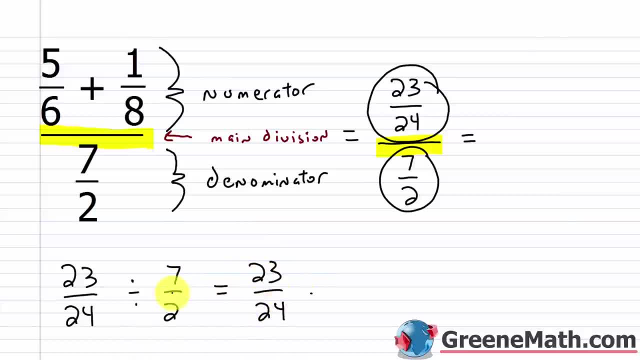 So this would be 23 over 24 times. flip this guy 2 over 7.. In this case you take again 23 over 24 times. take the reciprocal of the fraction on the bottom 2. sevenths: 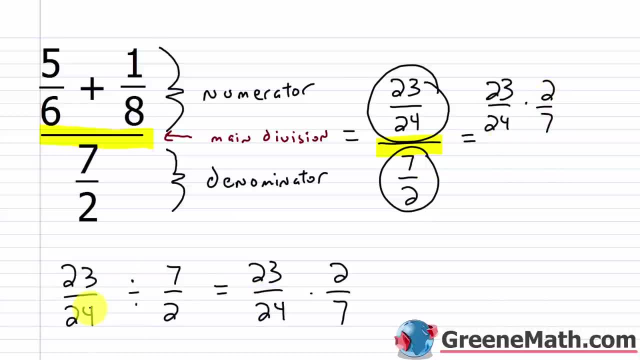 Either kind of way you want to do it, This is what we've been working with so far. This is kind of the new way that we're going to see kind of moving forward in math. So you know, I want you to get comfortable doing it in this way. 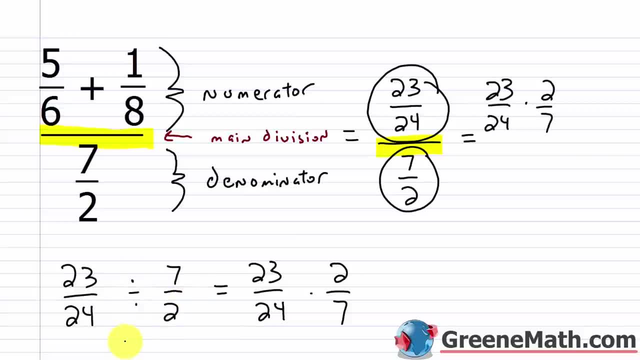 I know you're already comfortable doing it in this way. You know, if the first few times you do this you've got to convert it from this to this so that it makes sense for you in your mind, then go ahead and do it. 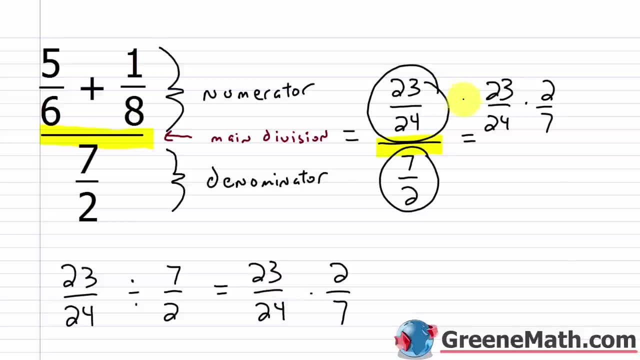 But after you know 10 or 15 problems or so, you want to try to merge into doing it this way because, again, as you move forward, this is going to be more common. Okay, so let me just erase this. 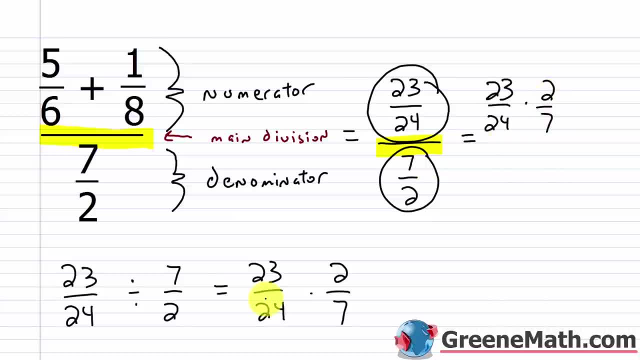 on the bottom 2 sevenths either kind of way you want to do it this is what we've been working with so far this is kind of the new way that we're going to see kind of moving forward in math so you know i want you to get comfortable doing it in this way i know you're already comfortable doing it in this way you know if the first few times you do this you've got to convert it from this to this so that it makes sense for you in your mind so go ahead and do it but after you know 10 or 15 problems or so you want to try to merge into doing it this way because again as you move forward this is going to be more common 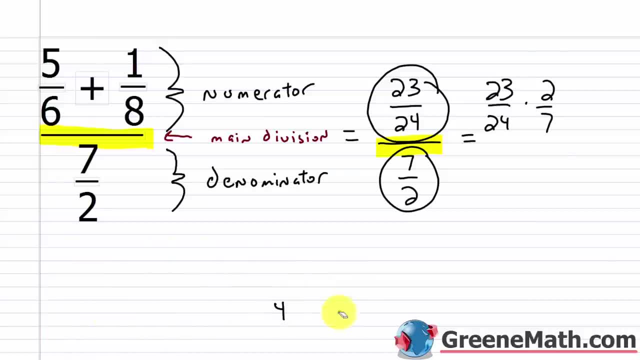 okay so let me just erase this we know how that sets up 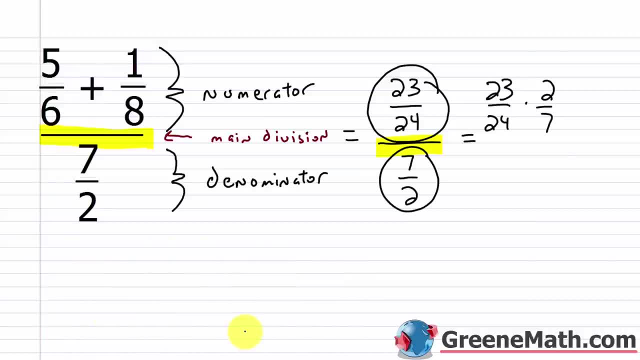 and what i want to do i want to cancel any common factors 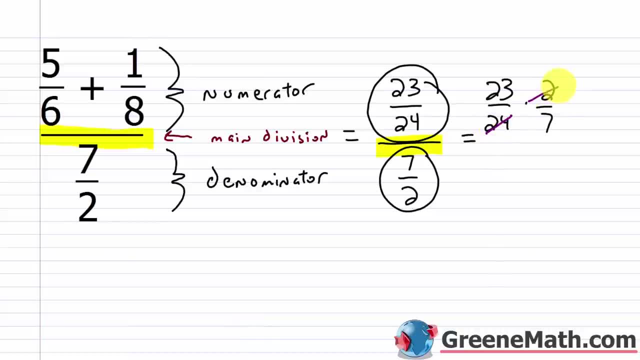 before i multiply so now i can cross cancel a 2 between here and here and this would be 12 so now what i'm going to be left with 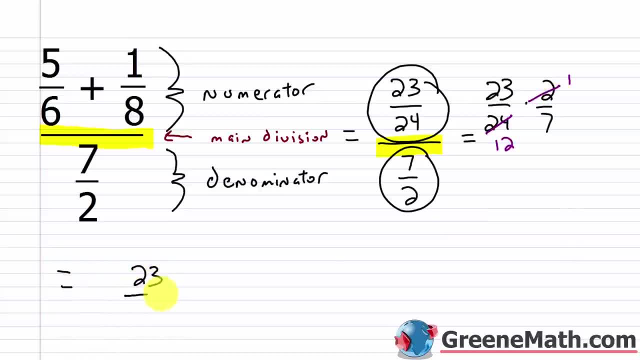 is a 23 times 1 for my simplified numerator over 12 times 7 which is 84 so i get 23 over 84 as the simplified complex fraction 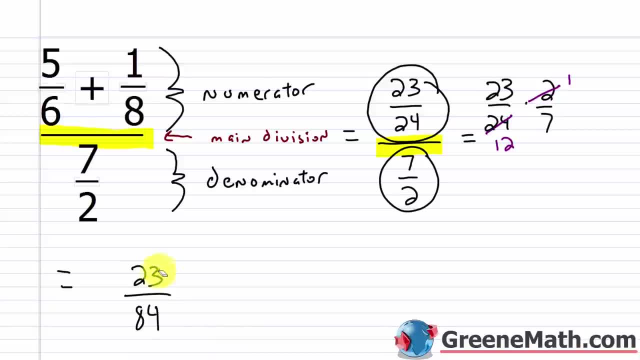 now i taught you another method to do this in the lesson let me erase all this and let me just kind of erase this real fast 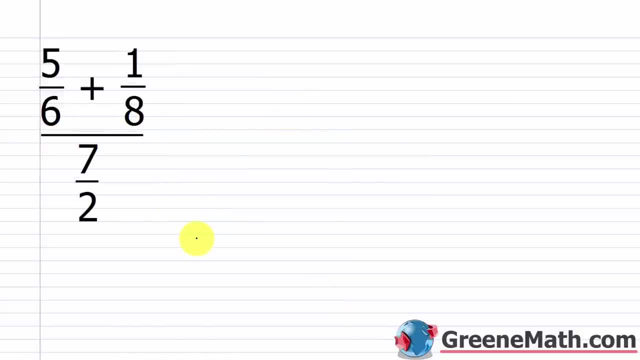 the other method is to multiply the numerator and the denominator of the complex fraction 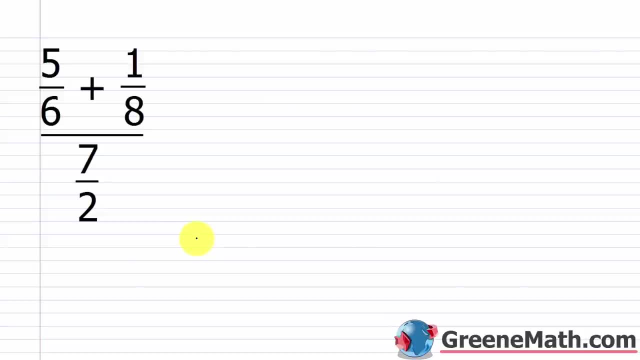 by the LCD of all denominators involved so in order to do that i'm going to do this i'm looking for the LCD i want to look at all the denominators 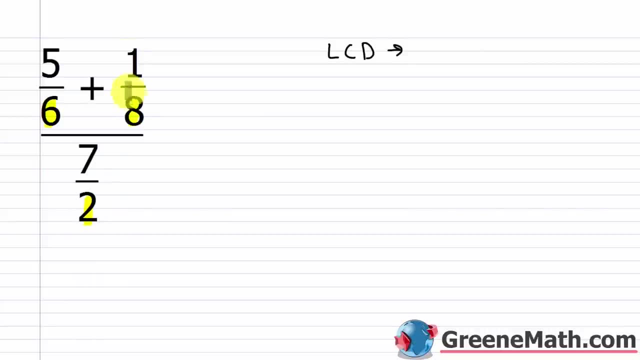 so i have a 6 here, an 8 here and a 2 here that's all the denominators that are involved in the complex fraction 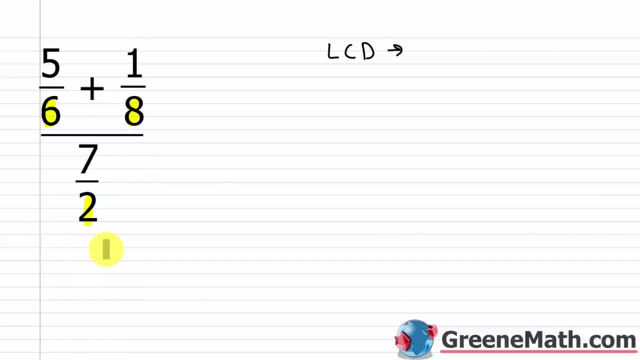 i'm not looking at just the denominator of the complex fraction 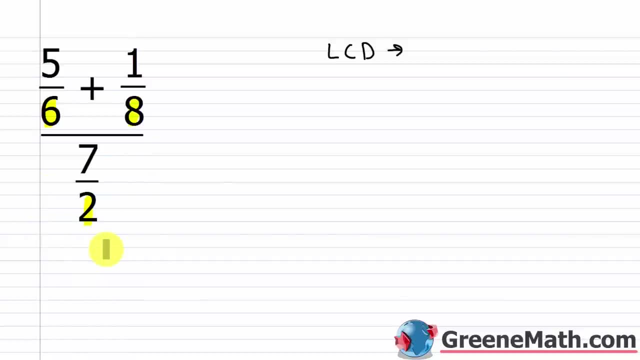 i'm looking at individually each denominator that's involved 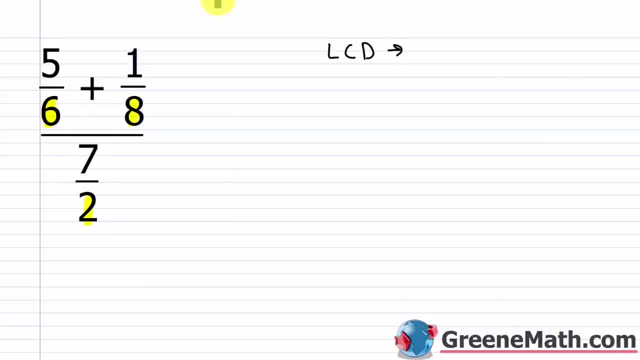 so kind of in the numerator if i was to block this out let me get a black color and just 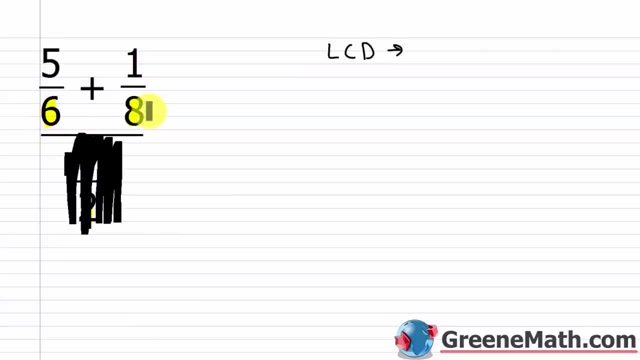 kind of block this out i have two denominators, i have a 6 and an 8 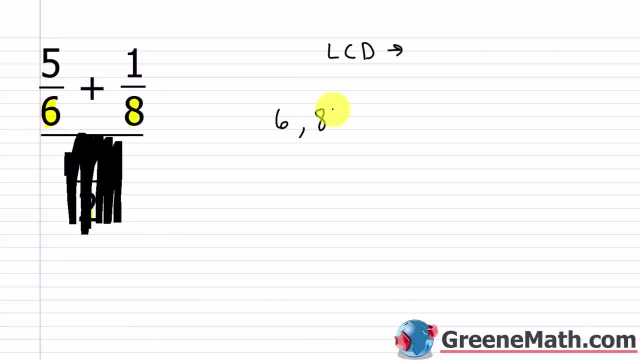 so i'm thinking about 6 and i'm thinking about 8 and then kind of if i look at my 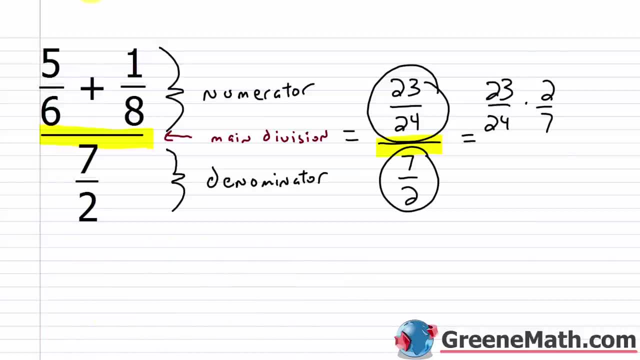 We know how that sets up And what I want to do. I want to cancel any common factors before I multiply, So now I can cross cancel a 2 between here and here, and this would be 12.. So now what I'm going to be left with is a 23 times 1 for my simplified numerator over 12 times 7, which is 84. 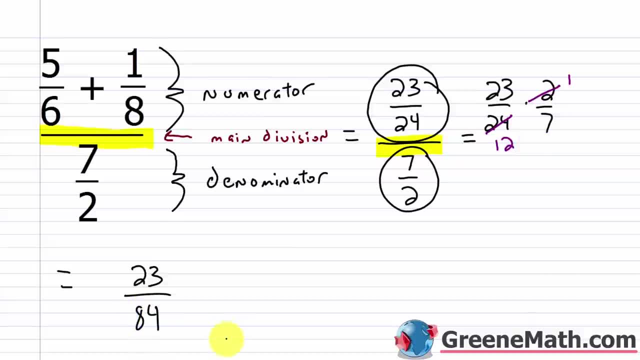 So I get 23 over 84 as the simplified complex fraction. Now I taught you another method to do this in the lesson. Let me erase all this And let me just kind of erase this real fast. The other method is to multiply the numerator and the denominator of the complex fraction by the LCD of all denominators involved. 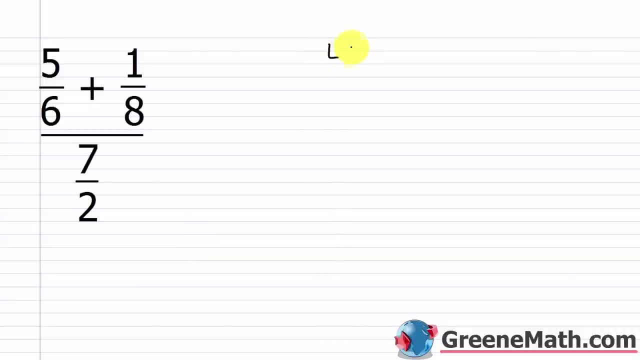 So in order to do this, I'm looking for the LCD. I want to look at all the denominators. So I have a 6 here, an 8 here and a 2 here. That's all the denominators that are involved in the complex fraction. 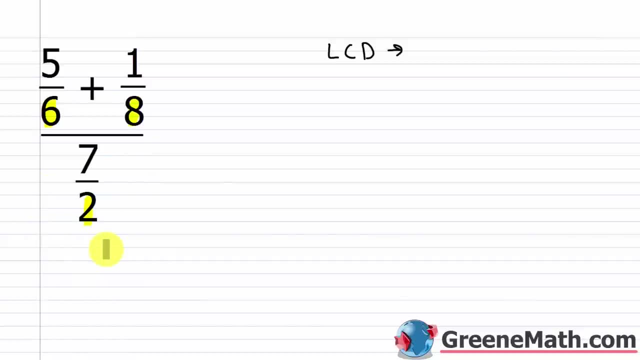 I'm not looking at just the denominator of the complex fraction. I'm looking at individually each denominator that's involved So kind of in the numerator. if I was to block this out, Let me get a black color and just kind of block this out. 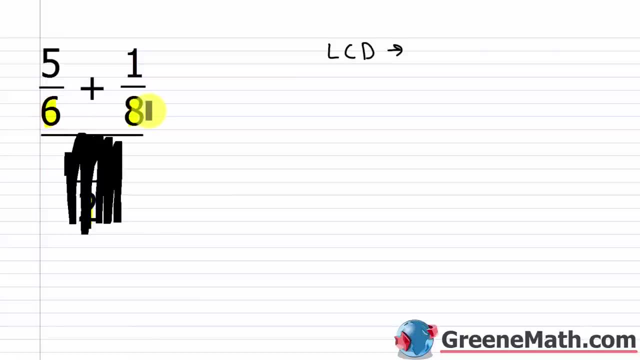 I have two denominators. I have a 6 and an 8. So I'm thinking about 6, and I'm thinking about 8. And then, kind of, if I look at my denominator of the complex fraction. Let me block this out for a minute. 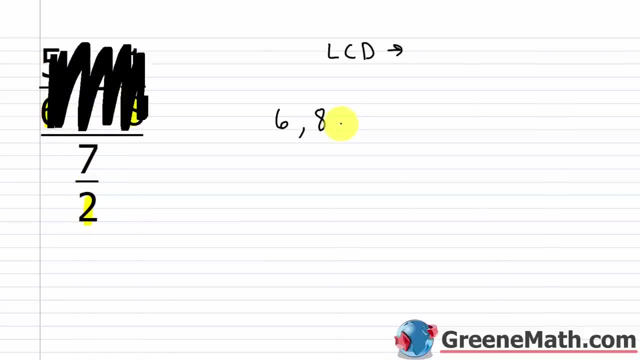 I have a denominator of 2.. So that's where I'm getting those numbers from. I don't want you to be confused. Now, once I have those numbers, I just find the least common denominator that I can form. Or again, that's the LCM, the least common multiple of these numbers. 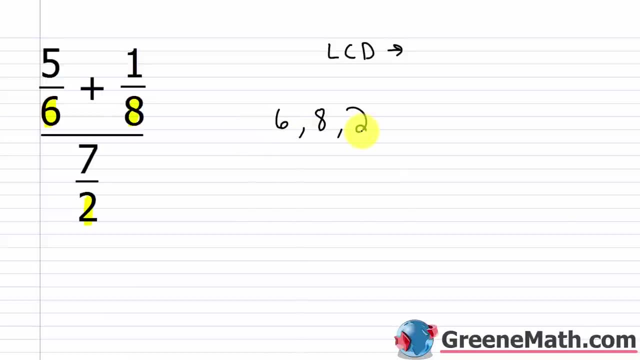 So what is the LCM of 6,, 8, and 2?? Well, I know that 2 doesn't factor. I know 8 is nothing more than 2 times 2 times 2.. And I know 6 is what. 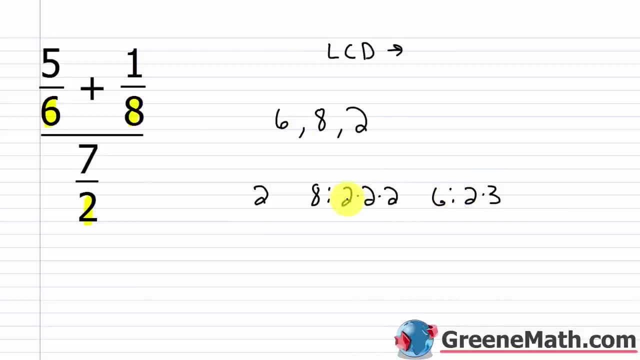 It's 2 times 3.. So it looks like we're going to have an LCD of 2 times 3. Or 8 times 3.. So that's going to be 24.. Now if I take 24, and again I multiply it by the numerator and denominator of the complex fraction, 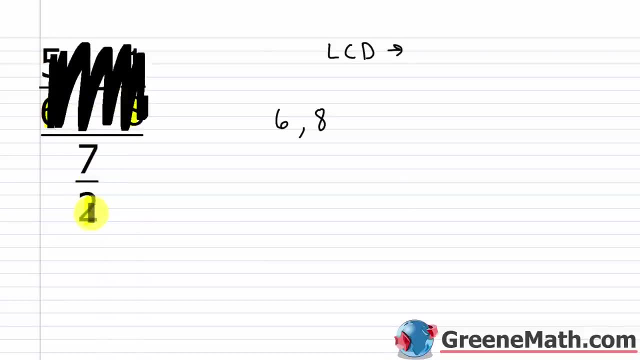 denominator of the complex fraction let me block this out for a minute i have a denominator of 2 so that's where i'm getting those numbers from 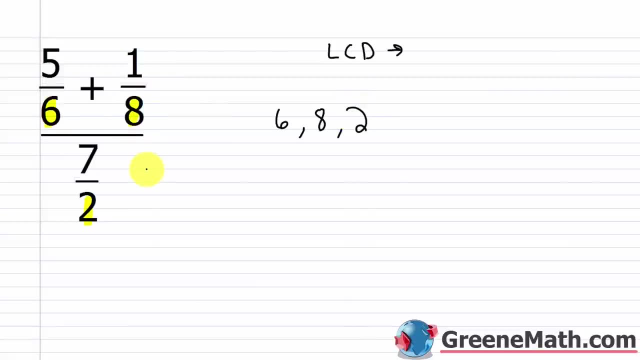 i don't want you to be confused now, once i have those numbers 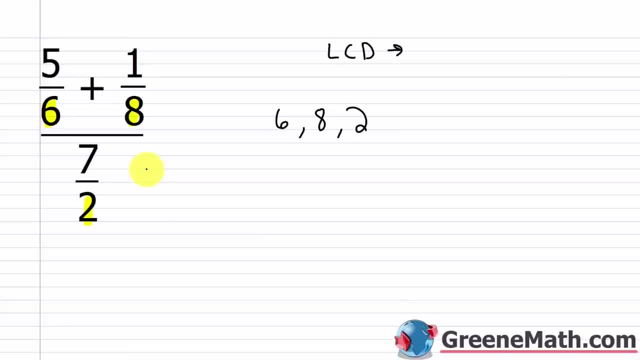 i just find the least common denominator that i can form or again, that's the LCM the least common multiple of these numbers so what is the LCM of 6, 8, and 2 well, i know that 6 is the length factor i know 8 is nothing more than 2 times 2 times 2 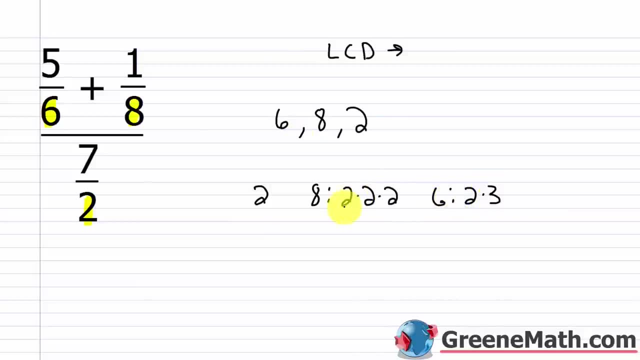 it's 2 times 3 so it looks like we're going to have an LCD of 2 times 2 times 2 or 8 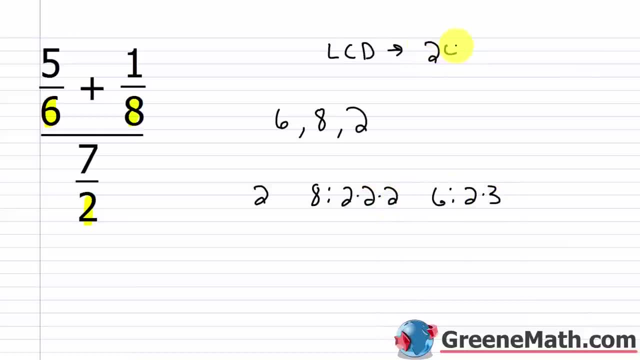 times 3 so that's going to be 24 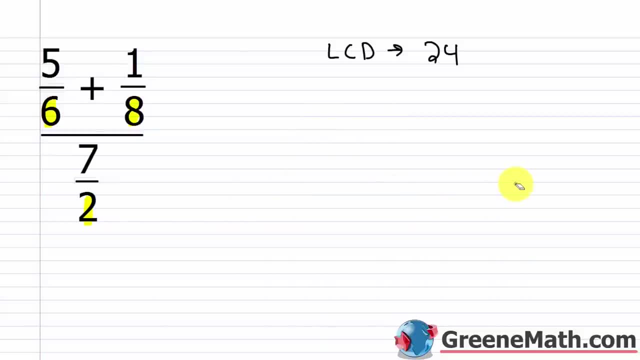 now if i take 24 and again i multiply it by the numerator and denominator of the complex fraction so i'm going to multiply this part right here by 24 and then this part right here by 24 what's going to happen i'm going to distribute this to each inside of the parentheses 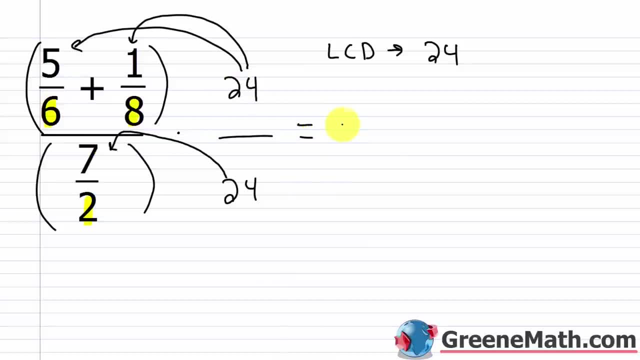 what am i going to get 24 times 5 is 6 let's do that over here this is going to cancel with this and give me a 4 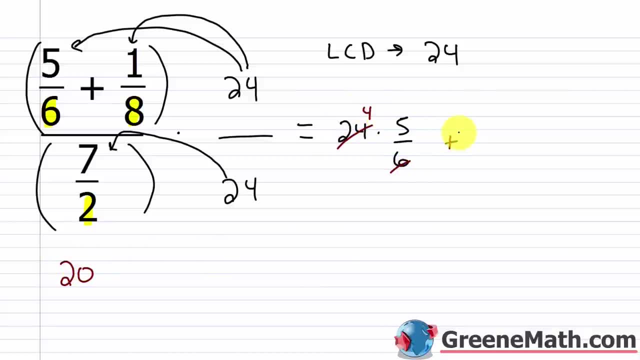 4 times 5 is 20 so let me write 20 over here 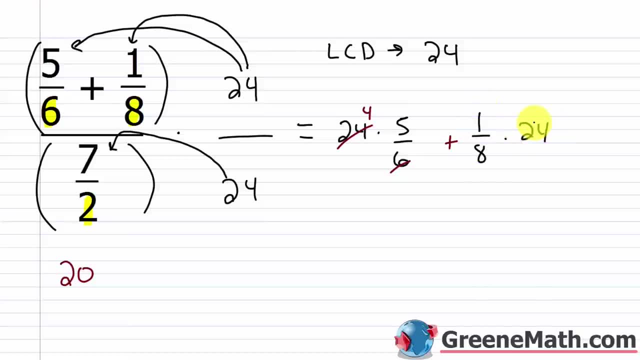 and then plus, i have 1 eighth times 24 and this is going to cancel with this 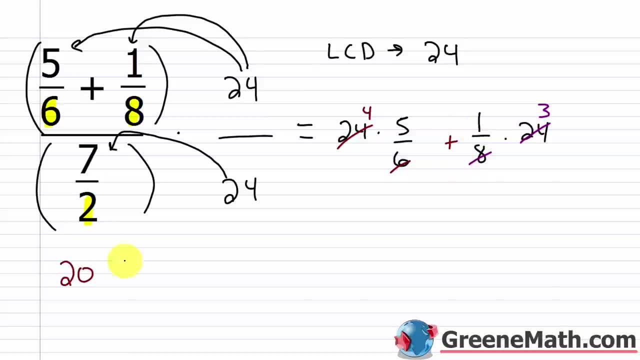 and give me a 3 plus 3 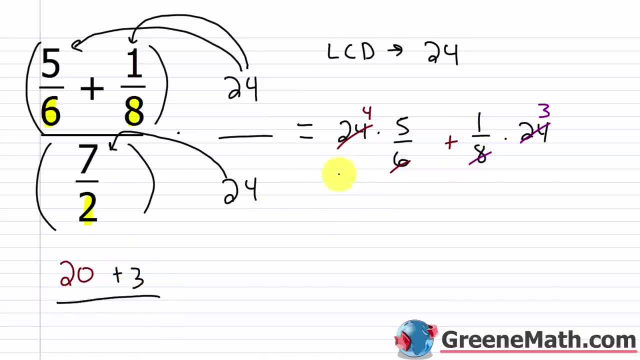 so then plus 3 and then over 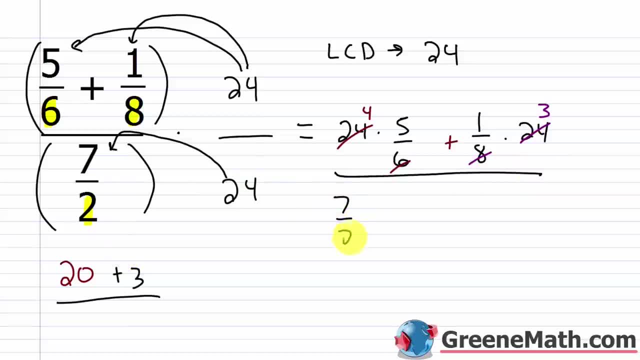 down here what i have is 24 times 7 halves so 7 halves times 24 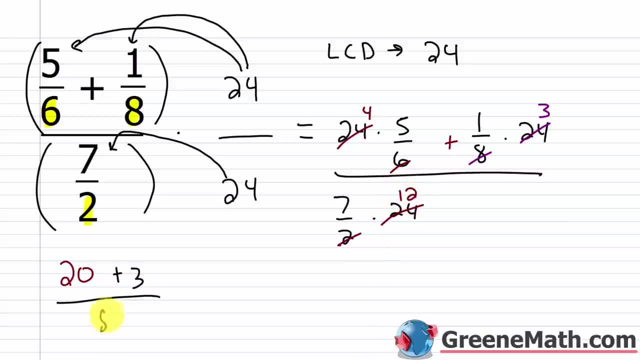 now we can see this would cancel with this and give me a 12 12 times 7 is 84 so this equals 20 plus 3 is 23 over 84 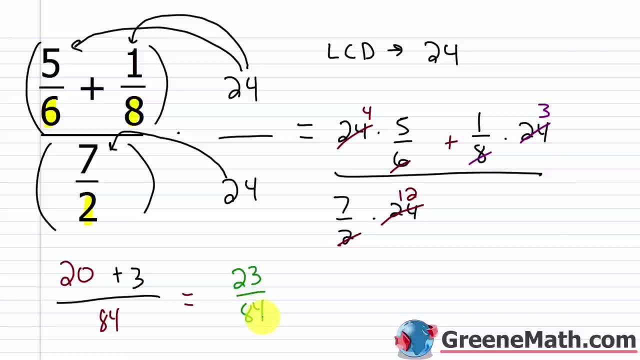 so i get the same answer either way it's just a different method and as far as which one you want to use just depends on you the lcd or understanding what i'm doing here you might want to do it the first way to kind of break it down 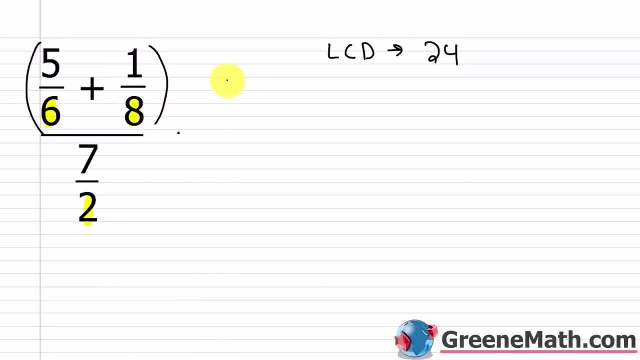 So I'm going to multiply this part right here by 24.. And then this part right here by 24.. What's going to happen? I'm going to distribute this to each inside of the parentheses. What am I going to do? What am I going to get? 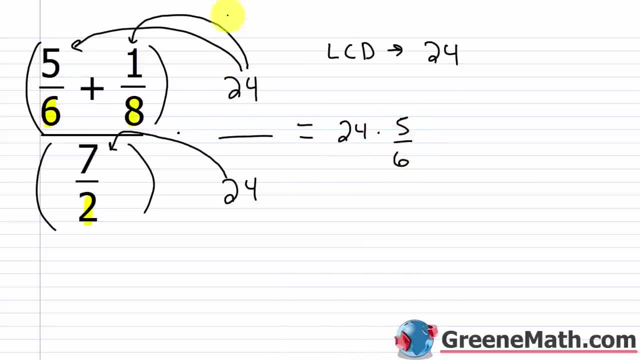 24 times 5 is 6.. Let's do that over here. This is going to cancel with this and give me a 4.. 4 times 5 is 20.. So let me write 20 over here, And then plus I have 1 eighth. 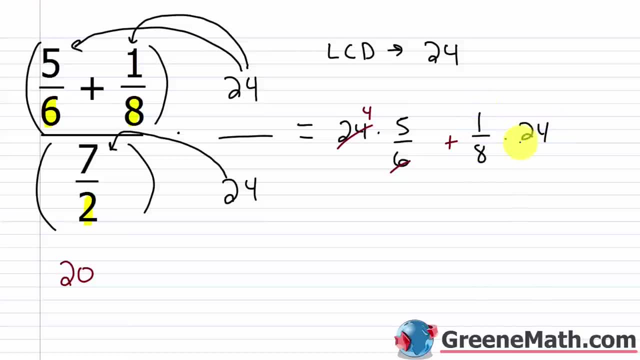 1, eighth times 24.. And this is going to cancel with this and give me a 3.. 3 times 1 is 3, so I'd have plus 3.. So then plus 3.. And then over down here what I have is 24 times 7 halves. 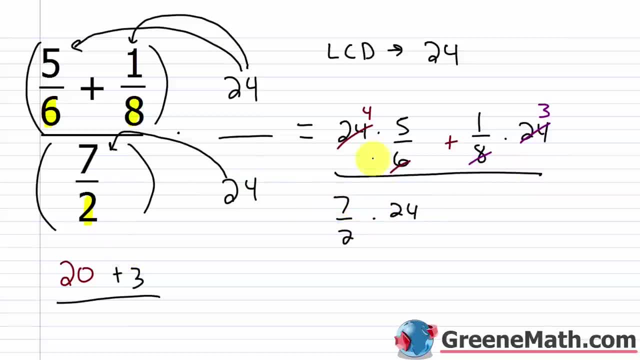 So 7 halves times 24. And we can see this would cancel with this and give me a 12.. 12 times 7 is 84. So this equals 20 plus 3 is 23 over 84. So I get the same answer either way. 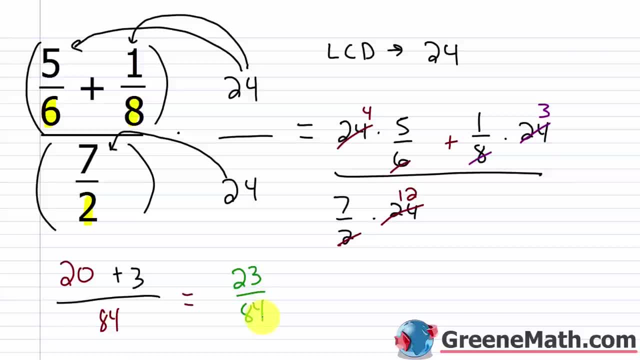 It's just a different method, And as far as which one you want to use, just depends on you. If you have trouble finding the LCD or understanding what I'm doing here, you might want to do it the first way to kind of break it down for yourself. 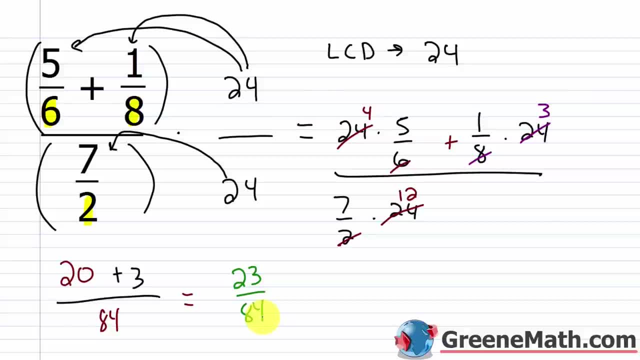 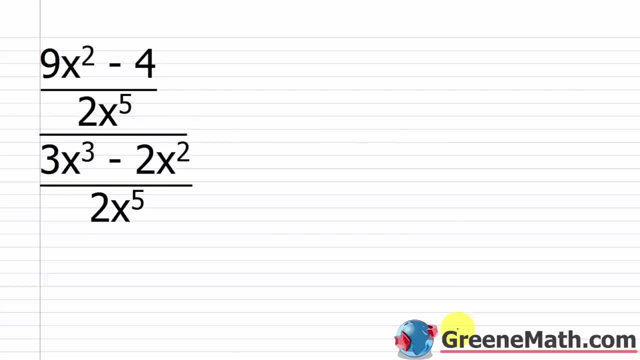 And then kind of move into this method as you get more comfortable. If you're completely comfortable with what I just did, then the LCD method is usually faster. Okay, so why are we talking about complex fractions again? Well, the reason that we're talking about complex fractions again. 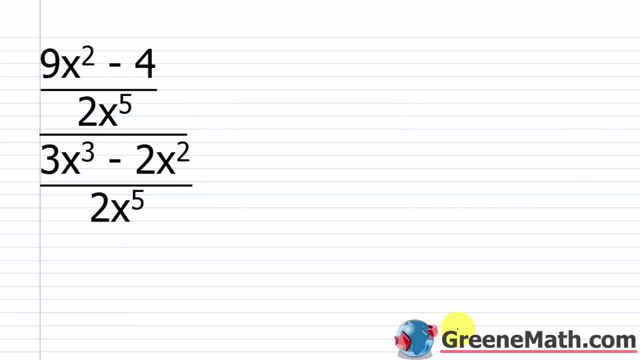 is because it comes up when you get to rational expressions Somewhere in your chapter. in rational expressions, usually right after you learn how to add and subtract, you're going to talk about complex fractions with regard to rational expressions, So it's the same thing. 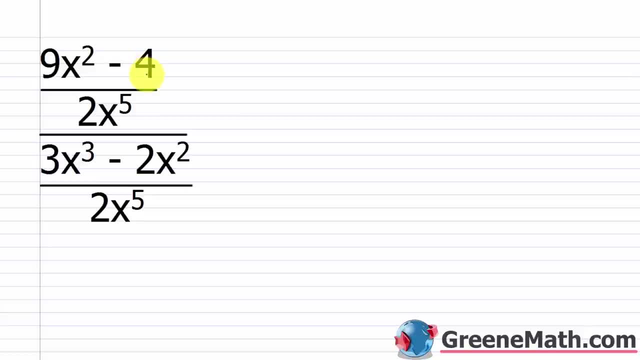 You have the same type of problem. It's just more complicated because there's variables involved, But you use the same methods to simplify. So, for example, if I have 9x squared minus 4 over 2x to the fifth power over 3x cubed minus 2x squared over 2x to the fifth power, 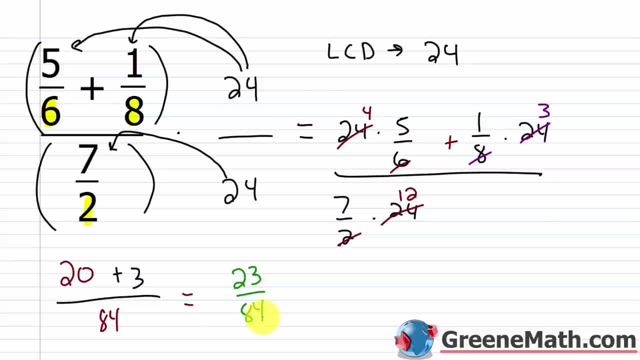 for yourself and then kind of move into this method as you get more comfortable if you're completely comfortable with what i just did then the lcd method is usually faster 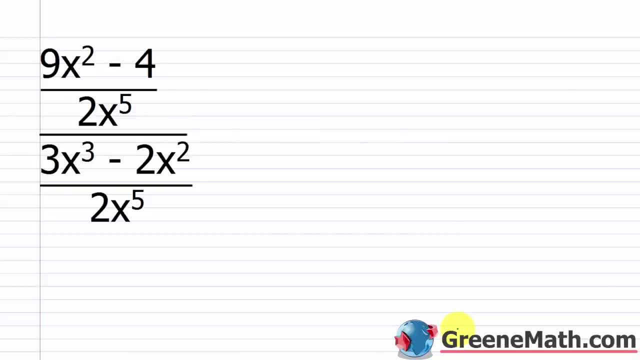 okay so why are we talking about complex fractions again well the reason that we're talking about complex fractions again is because it comes up when you get to rational expressions somewhere in your chapter on rational expressions usually right after you learn how to add and subtract you're going to talk about complex fractions with regard to rational expressions so it's the same thing you have 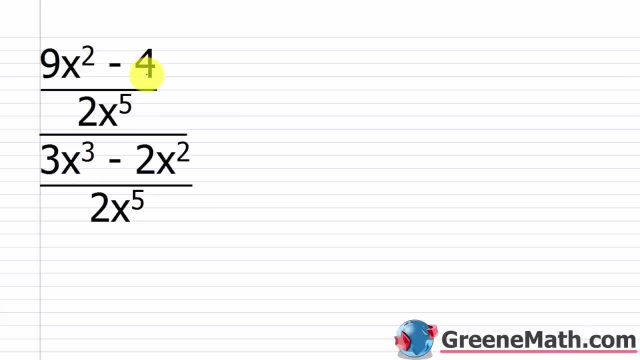 the same type of problem it's just more complicated because there's variables involved but you use the same methods to simplify 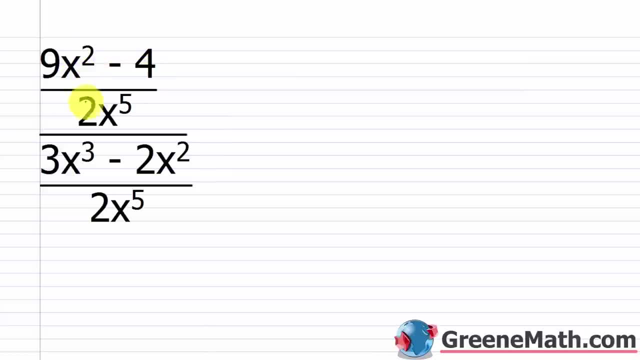 so for example if i have 9x squared minus 4 over 2x to the 5th power over 3x cubed minus 2x squared over 2x to the 5th power let's solve this guy just using kind of the first method 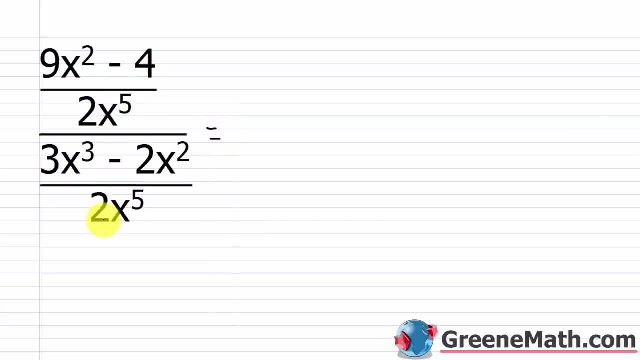 and what i want to do here is just simplify everything completely before i kind of set up the division so in the numerator here i have 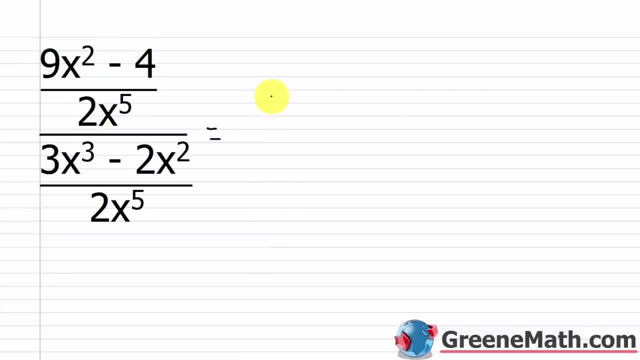 9x squared minus 4 the trick here is just try to factor everything before you get started to see what can factor and the trick with rational expressions is always to factor as you're working right you want to end up seeing what you can cancel 9x squared minus 4 i know that's the difference of two squares that is 3x plus 2 times 3x minus 2 then this is over 2x to the 5th power now i'm dividing by or my main division 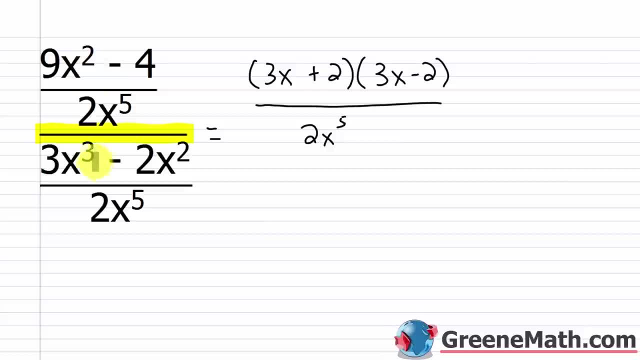 is here this is the numerator of the complex fraction this is the denominator so i would be multiplying by the reciprocal of this so then the denominator here in this denominator of the complex fraction i know that gets confusing but this is your denominator for the denominator of the complex fraction for this guy that is going to come up here 2x to the 5th power then the numerator is going to come down here but i see that i can 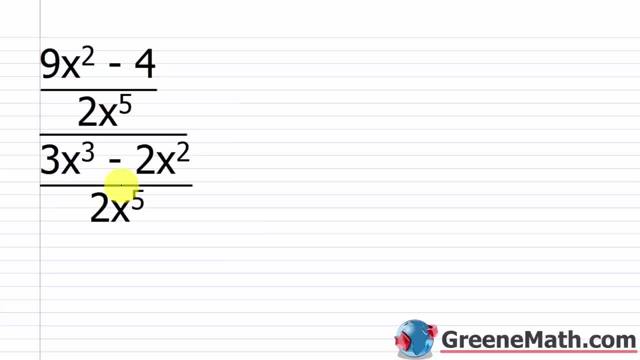 let's solve this guy just using kind of the first method, And what I want to do here is just simplify everything completely before I kind of set up the division. So in the numerator here I have 9x squared minus 4.. The trick here is just try to factor everything. 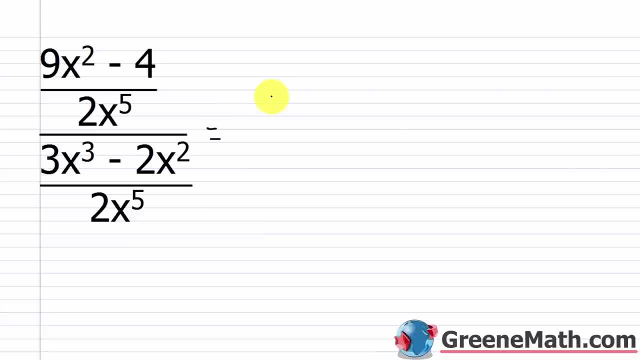 before you get started to see what can factor- And the trick with rational expressions is always to factor. as you're working- You want to end up seeing what you can cancel. 9x squared minus 4, I know that's the difference of two squares. 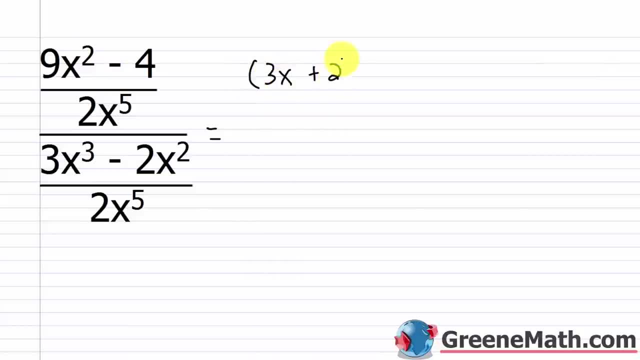 That is 3x plus 2 times 3x minus 2.. Then this is over 2x to the fifth power. Now I'm dividing by, or my main division is here. This is the numerator of the complex fraction. 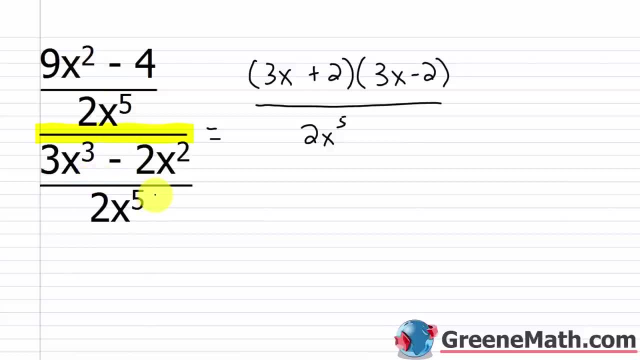 This is the denominator, So I would be multiplying by the reciprocal of this. So then, the denominator here in this denominator of the complex fraction. I know that gets confusing, but this is your denominator for the denominator of the complex fraction for this guy. 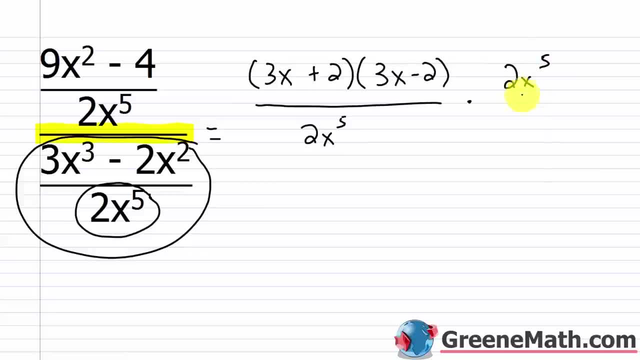 That is going to come up here. 2x to the fifth power, Then the numerator is going to come down here. But I see that I can factor out an x squared, So let me just go ahead and do that real quick. So x squared times if I pulled that out. 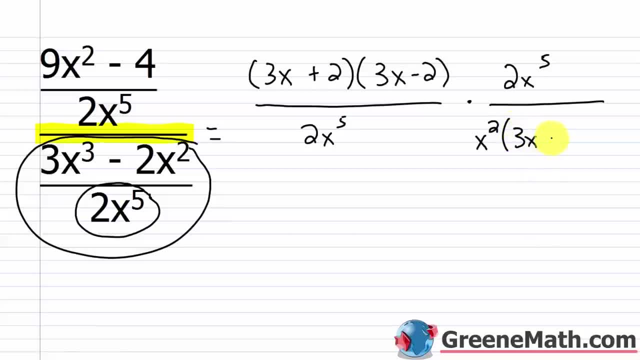 3x cubed, divided by x, squared would be 3x. And then minus 2x squared. divided by x, squared would be 2.. Now, before I do this multiplication, what can I cancel? I can cancel this factor of 3x minus 2. 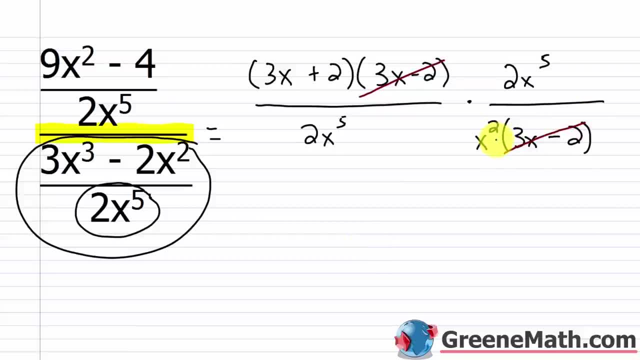 with this factor of 3x minus 2.. Remember, this is multiplication, here Multiplication. So these are factors. Now I can also cancel this 2x to the fifth power with this 2x to the fifth power, And what am I going to be left with? 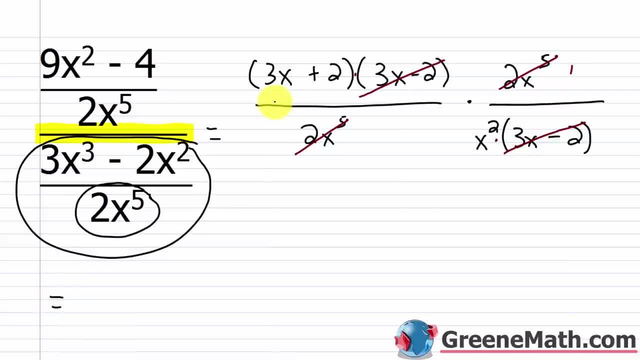 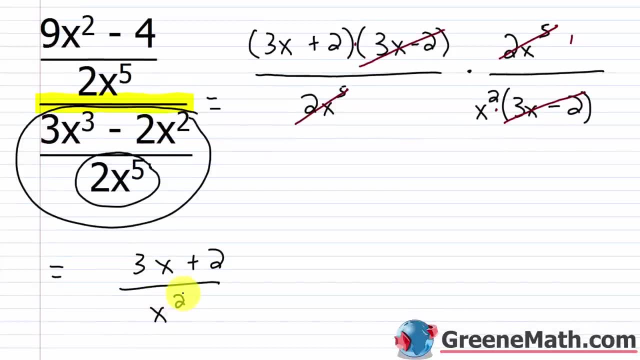 Well, I'm just going to have a 3x plus 2 in the numerator, over x squared in the denominator. So not too bad overall And this is kind of an easier example. And not that they get harder, They just get much, much more tedious. 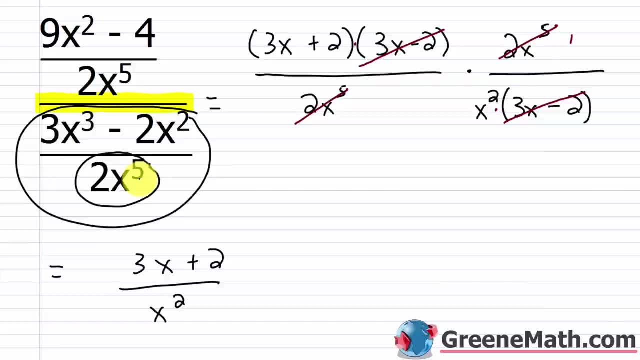 That's the trick. It just gets much, much more tedious, And so you need to take your time and go step by step so you don't make any silly mistakes. And just one more thing before I kind of get to the next problem. 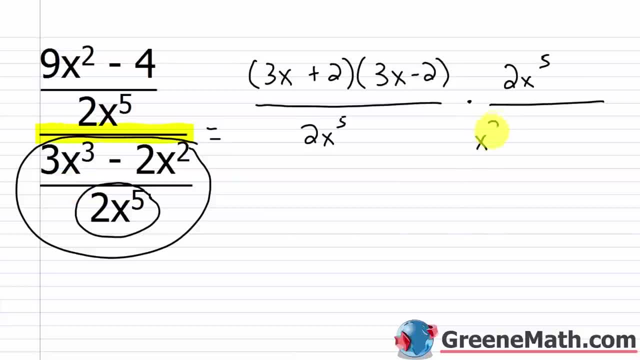 factor out an x squared so let me just go ahead and do that real quick so x squared times if i pulled that out 3x cubed divided by x squared would be 3x and then minus 2x squared divided by x squared would be 2 now before i do this multiplication what can i cancel i can cancel this factor of 3x minus 2 with this factor of 3x minus 2 remember this is multiplication here multiplication so these are factors 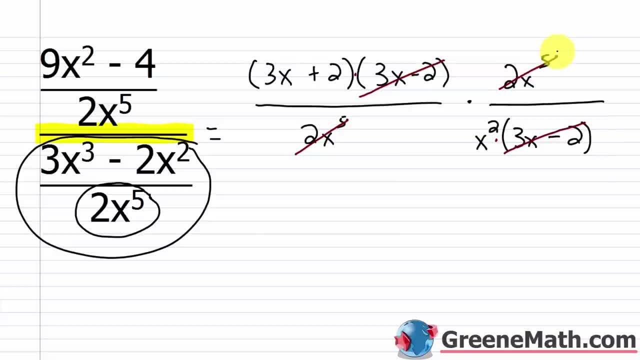 now i can also cancel this 2x to the 5th power with this 2x to the 5th power and what am i going to be left with well i'm just going to have a 3x plus 2 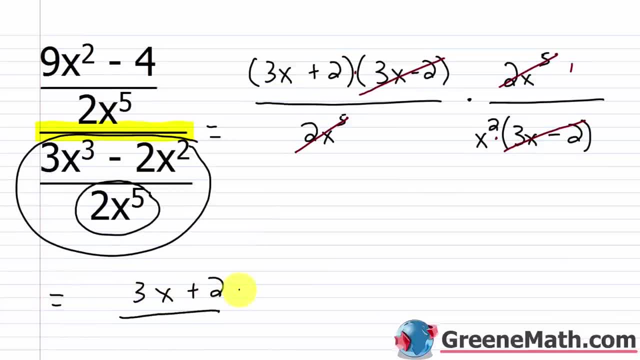 in the numerator over x squared in the denominator 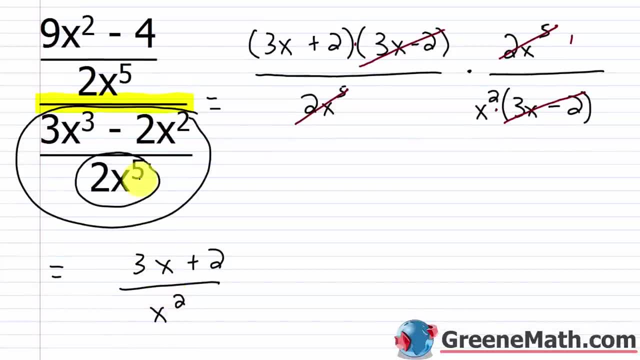 so not too bad overall and this is kind of an easier example and not that they get harder they just get much much more tedious right that's the trick it just gets much much more tedious and so you need to take your time and go step 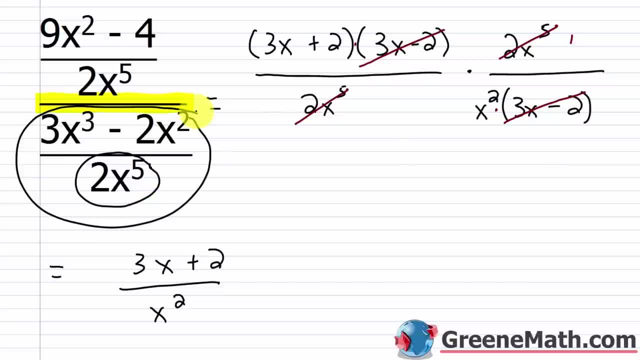 by step so you don't make any silly mistakes and just one more thing before i kind of get to the next problem again when you see your main division if you're uncomfortable setting it up like this go ahead and take this guy and say okay i have 3x plus 2 times 3x minus 2 over you know 2x to the 5th power take your main division and put a division symbol out there keep this as it is so i would factor out the x squared and then have 3x minus 2 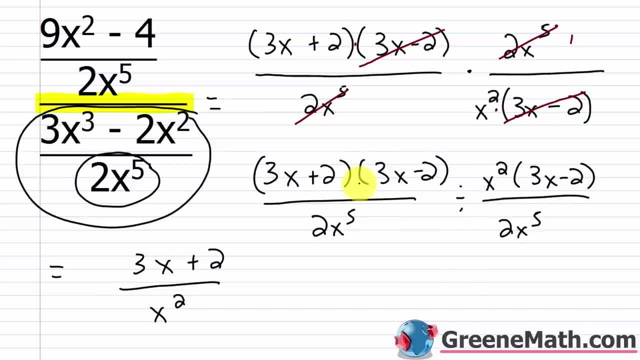 and then over 2x to the 5th power when i set it up like this it reminds me 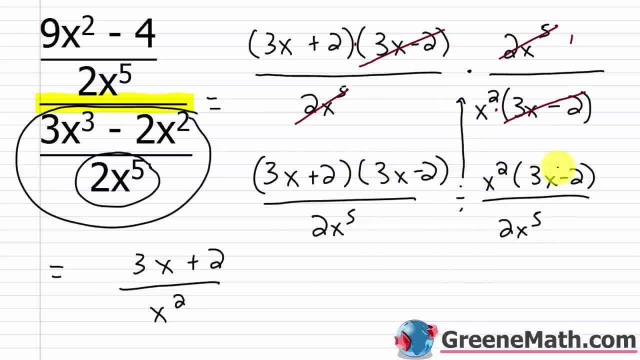 to multiply this guy right here by the reciprocal of this guy i set it up in one step here 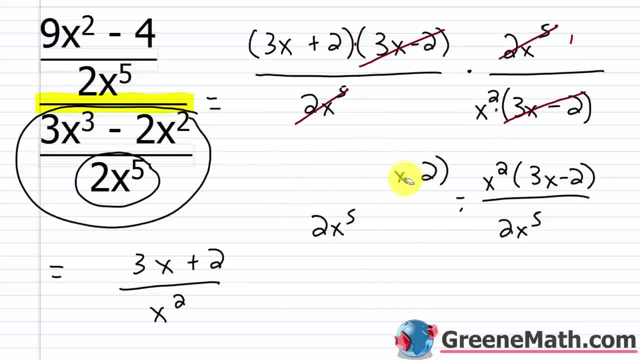 but again it might take you two because you might be so used to kind of doing that from prealgebra and that's fine again 10 or 15 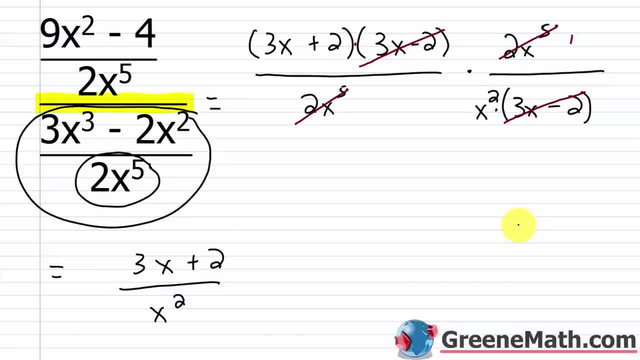 problems go by you want to kind of just convert to the new method because again as we move forward in math we're going to see it more and more as this versus what we 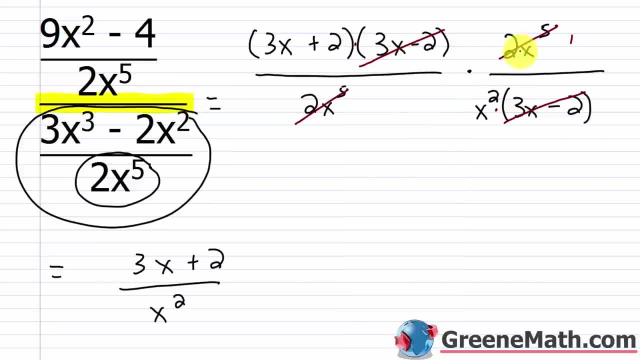 Again, when you see your main division, if you're uncomfortable setting it up like this, go ahead and take this guy and say, okay, I have 3x plus 2 times 3x minus 2 over, you know, 2x to the fifth power. 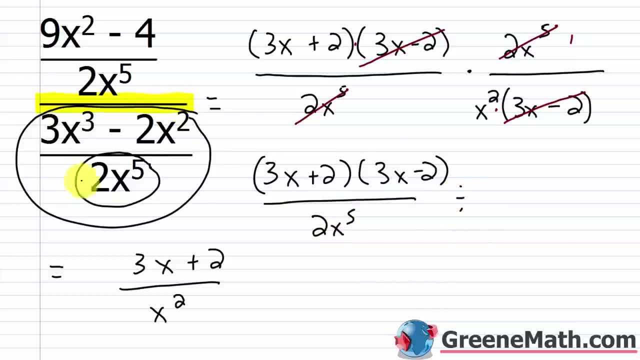 Take your main division and put a division symbol out there. Keep this as it is. So I would factor out the x squared and then have 3x minus 2, and then over 2x to the fifth power. When I set it up like this: 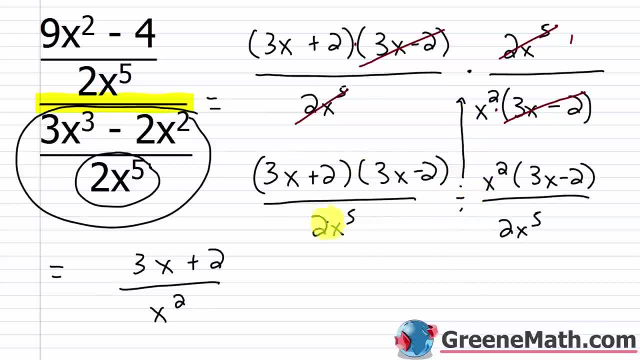 it reminds me to multiply this guy right here by the reciprocal of this guy. I set it up in one step here, But again it might take you two because you might be so used to kind of doing that from pre-algebra, And that's fine. 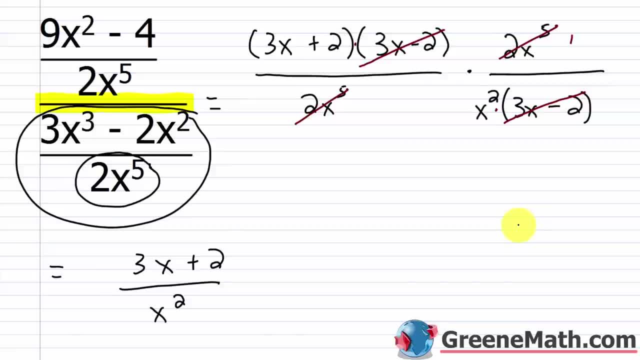 Again, 10 or 15 problems go by. You want to kind of just convert to the new method because again, as we move forward in math, we're going to see it more and more as this versus what we saw back in pre-algebra. 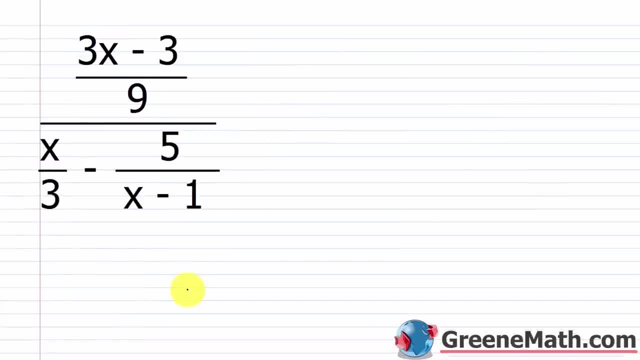 All right, let's take a look at another one. So I have 3x minus 3 over 9, and then this is over x over 3 minus 5 over x minus 1.. So again, what I'm going to do is use that kind of first method. 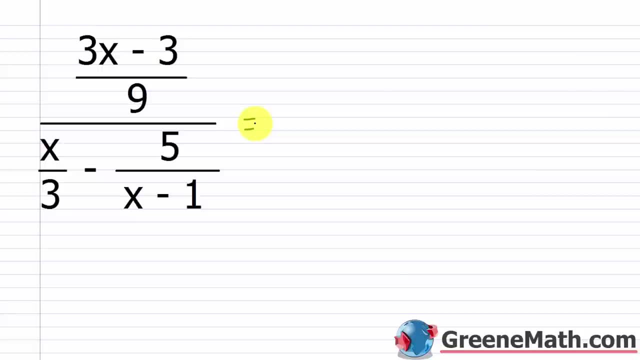 where I simplify the numerator and denominator completely, Then I kind of perform the main division. So the first thing I would do is I would just find the main division bar. So this is the numerator of the complex fraction, This is the denominator, That's your main division. 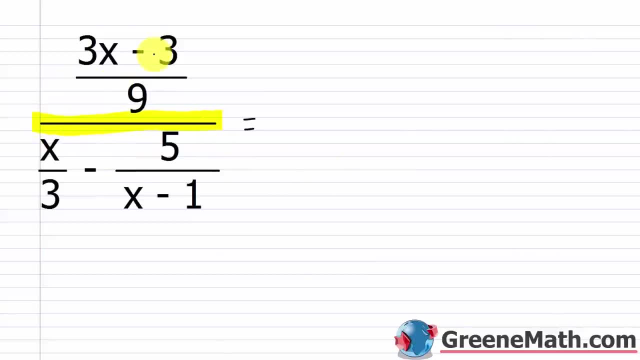 Okay, So for the numerator, is there anything I can do to simplify that? Well, 3x minus 3, I could factor out a 3, and I'd have x minus 1 inside the parentheses. This is over 9.. 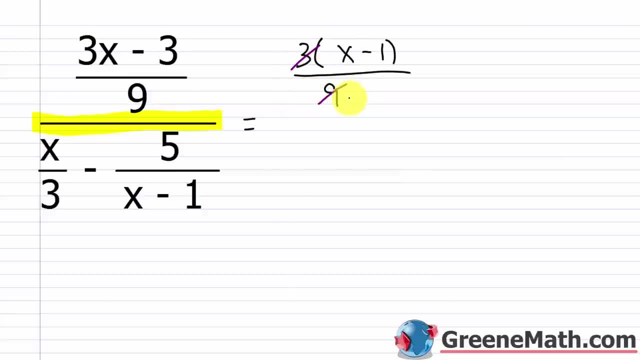 3 and 9 share a common factor of 3.. So this can be canceled. with this, This would be a 3, and this would be a 1.. Now, this is over. For this one, I have to do a little bit more work. 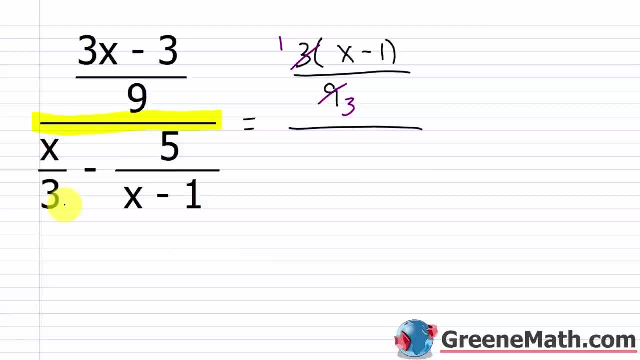 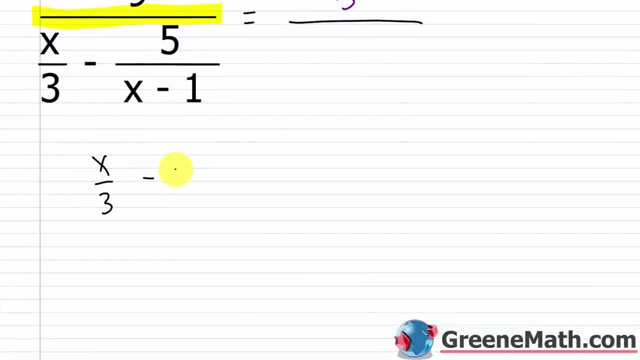 I have x over 3 minus 5 over x minus 1.. Now let me kind of scroll down a little bit and let me do this down here. So x over 3 minus 5 over x minus 1.. What would the LCD be? 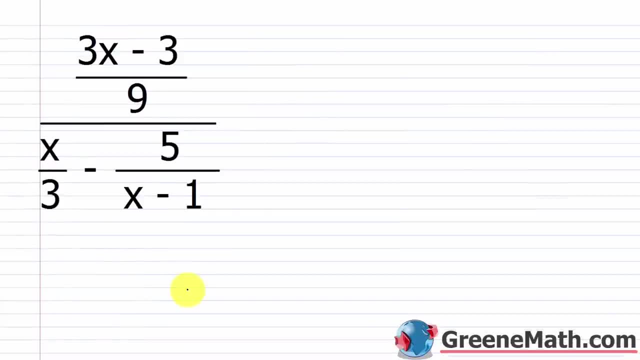 saw back in prealgebra alright let's take a look at another one so i have 3x minus 3 over 9 and then this is over x over 3 minus 5 over x minus 1 so again what i'm going to do is use that kind of first method where i simplify the numerator and denominator completely then i kind of perform the main division so the first thing i would do is i would just find the main division bar so this is the numerator of the complex fraction this is the denominator that's your main division ok so for the 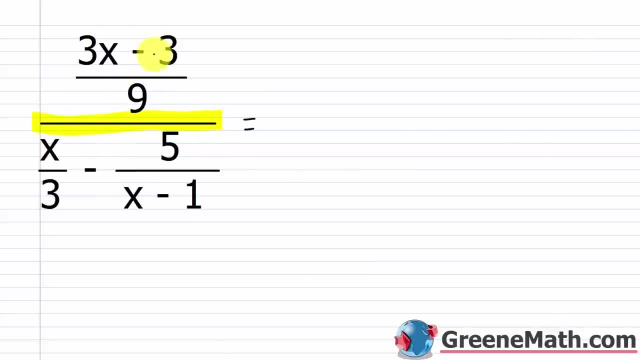 numerator is there anything i can do to simplify that well 3x minus 3 i could factor out a 3 and i'd have x minus 1 inside the parenthesis this is over 9 3 and 9 share a common factor of 3 so this can be cancelled with this this would be a 3 and this would be a 1 now this is over for this one i have to 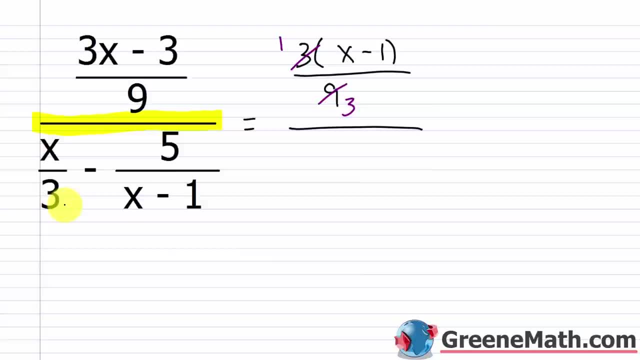 do a little bit more work and x over 3 minus 5 over x minus 1 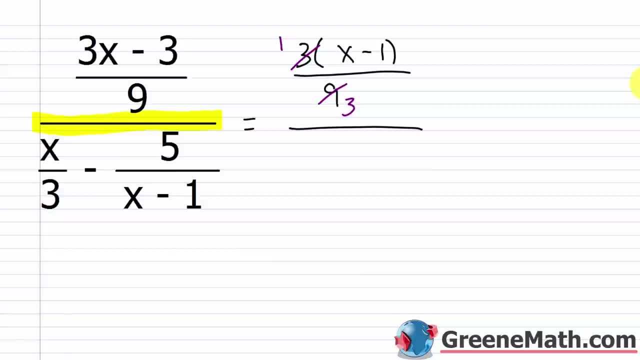 now let me kind of scroll down a little bit and let me do this down here 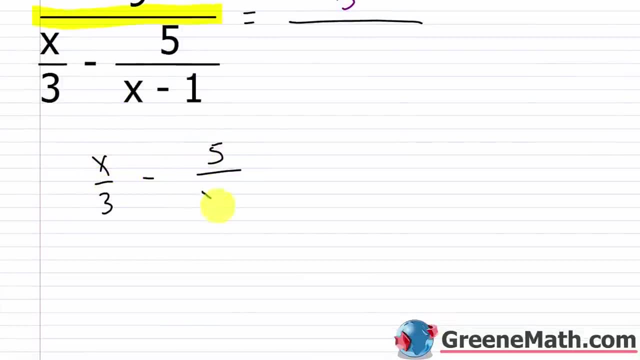 so x over 3 minus 5 over x minus 1 what would the lcd be well it would just be 3 times the quantity x minus 1 so i would multiply this by 3 over 3 and i would multiply this by x minus 1 over x minus 1 and what would that give me x times x is x squared minus x times 1 is x and then minus 3 times 5 is 15 then this is over that lcd of 3 times 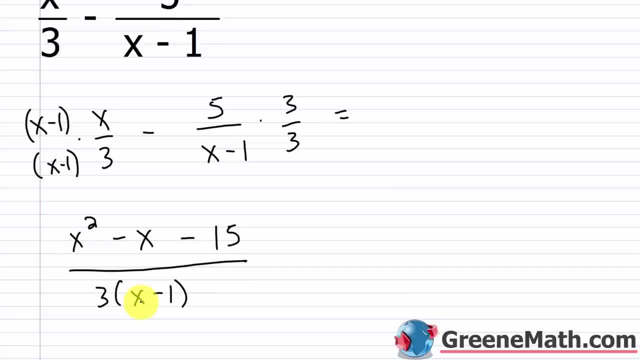 the quantity x minus 1 and i'm not going to multiply it i'm just going to leave it in factored form for right now 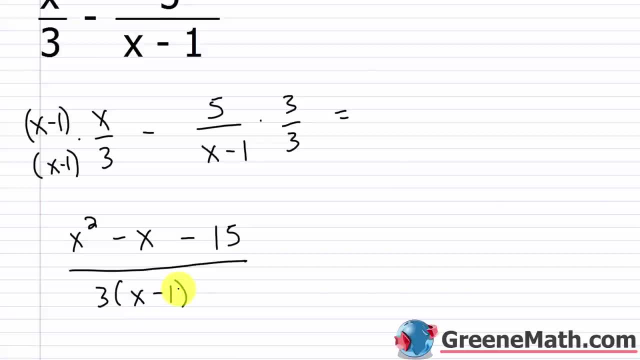 just in case it will cancel with something later on you don't want to go through a multiply and then have to go back and factor you want to save yourself a little bit of work 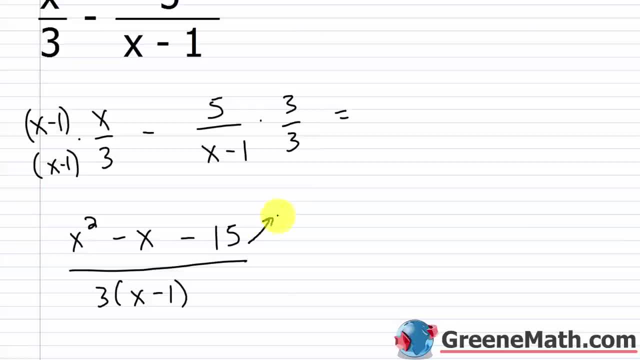 can i factor x squared minus x minus 15 into the product of two binomials well this would be x and this would be x can you 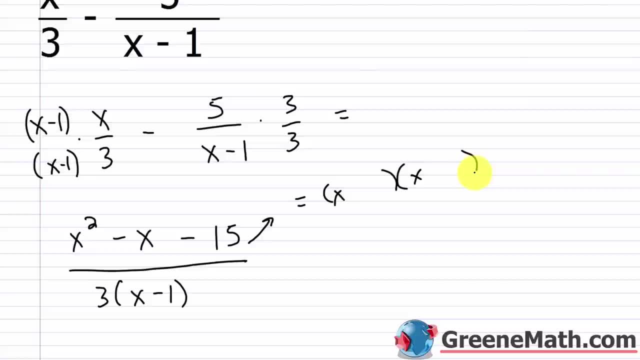 give me two integers whose product is negative 15 and whose sum is negative 1 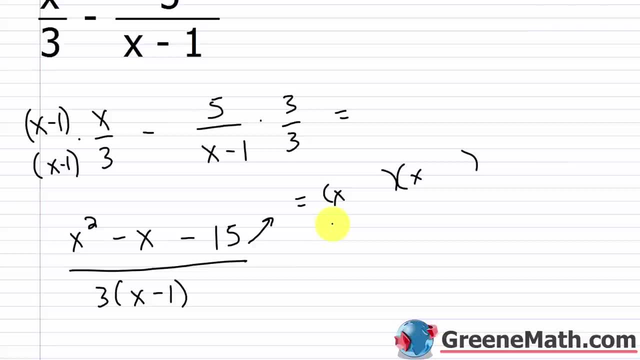 well 15 only factors into 1 times 15 or 5 times 3 so no that's not going to be possible so this is going to be prime 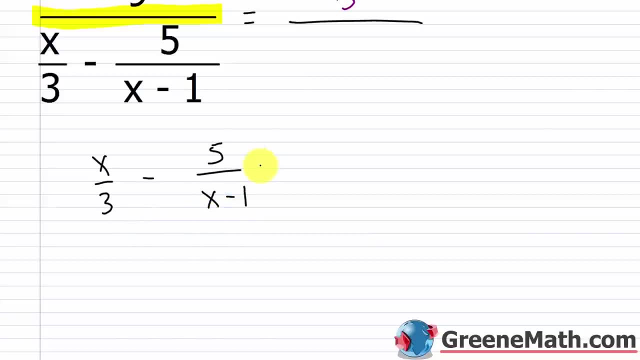 Well, it would just be 3 times the quantity x minus 1.. So I would multiply this by 3 over 3, and I would multiply this by x minus 1 over x minus 1.. And what would that give me? 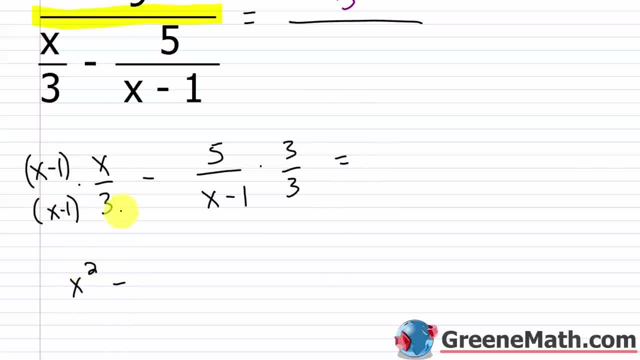 x times x is x. squared minus x times 1 is x, And then minus 3 over 3.. 3 times 5 is 15.. Then this is over that LCD of 3 times the quantity x minus 1.. And I'm not going to multiply it. 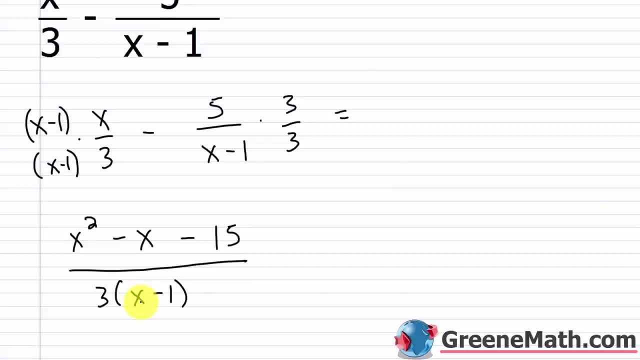 I'm just going to leave it in factored form for right now, just in case it will cancel with something later on. You don't want to go through a multiply and then have to go back and factor. You just want to save yourself a little bit of work. 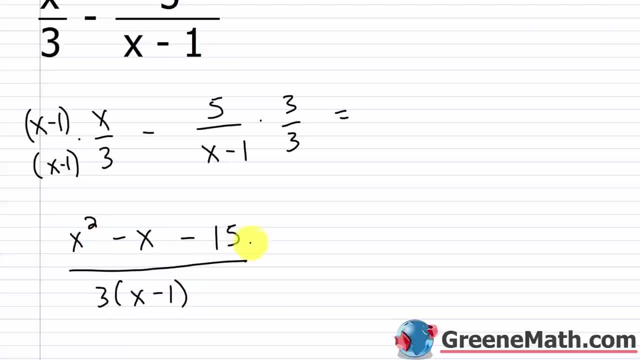 Can I factor x, squared minus x minus 15, into the product of two binomials? Well, this would be x and this would be x. Can you give me two integers whose product is negative 15 and whose sum is negative 1?? 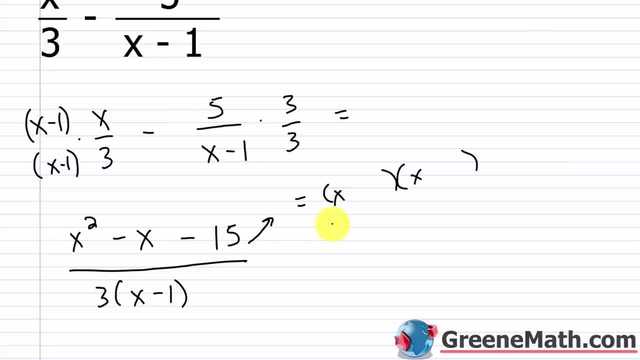 Well, 15 only factors into 1 times 15 or 5 times 3.. So, no, that's not going to be possible. So this is going to be prime, And so I'm going to drag this back up to the top. 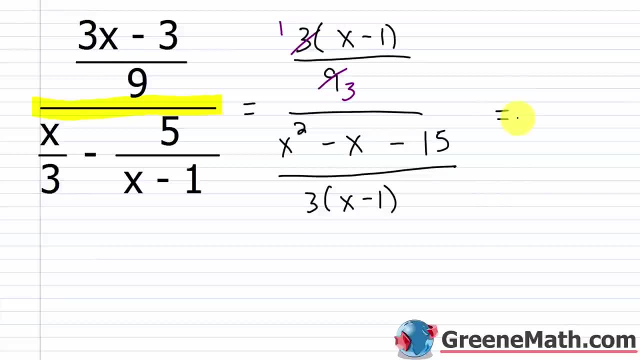 And now I'm going to go ahead and set up my multiplication. So I have the numerator here, or the top part, as x minus 1, that quantity over 3.. And then I have my denominator down here, which I'm going to flip it right. 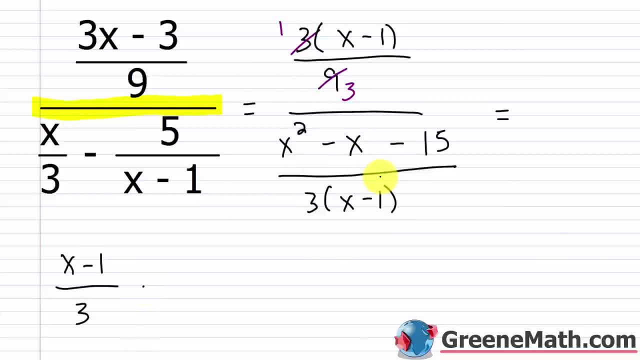 I'm going to take the top part, multiply it by the reciprocal of the bottom part. So we would have 3 times the quantity x minus 1 on the top over x squared minus x minus 15 on the bottom. So is there anything I can cancel before I do the multiplication? 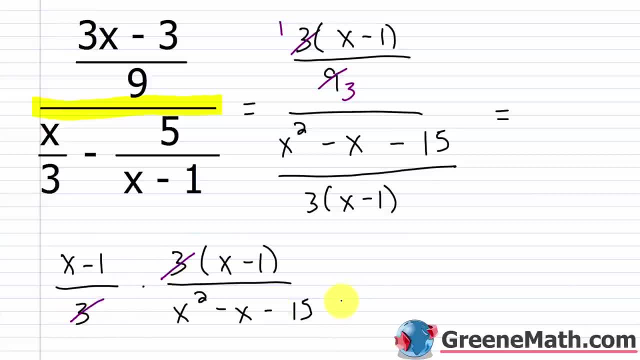 This 3 with this 3. And then that's it. So what I'm left with is x minus 1, that quantity times x minus 1. again We could say that's x minus 1 squared, if we want. 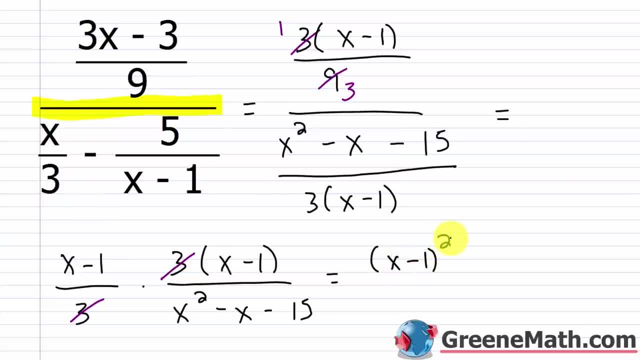 Or your teacher might want you to go through and actually do the FOIL, you know, just to get some practice. That's fine. And then this is over: x squared minus x minus 15.. And just for the sake of completeness, let's go ahead and do that. 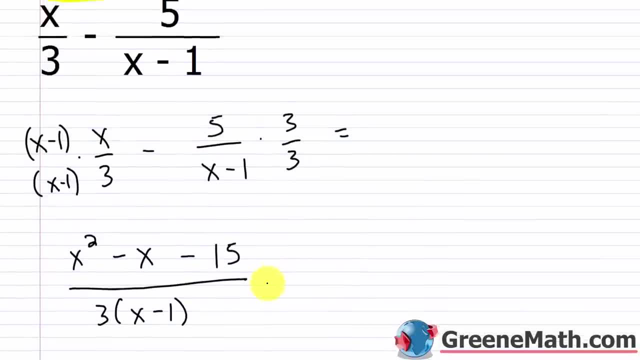 and so i'm going to drag this back up to the top 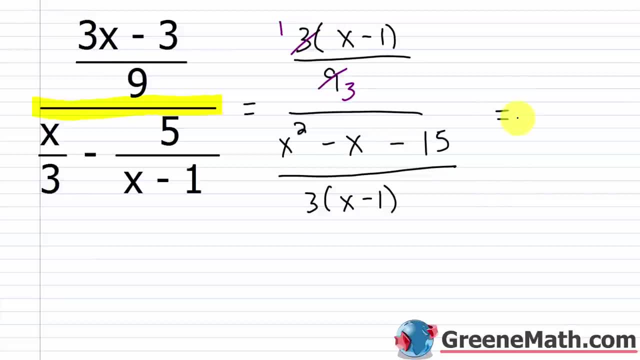 and now i'm going to go ahead and set up my multiplication so i have the numerator here or the top part as x minus 1 that quantity over 3 and then i have my denominator down here which i'm going to flip it right i'm going to take the top part multiply it by the 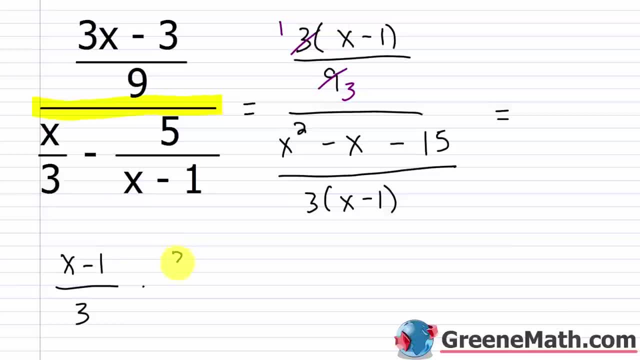 reciprocal of the bottom part so we would have 3 times the quantity x minus 1 on the top over x squared minus x minus 15 on the bottom so is there anything i can cancel before i do the multiplication this 3 with this 3 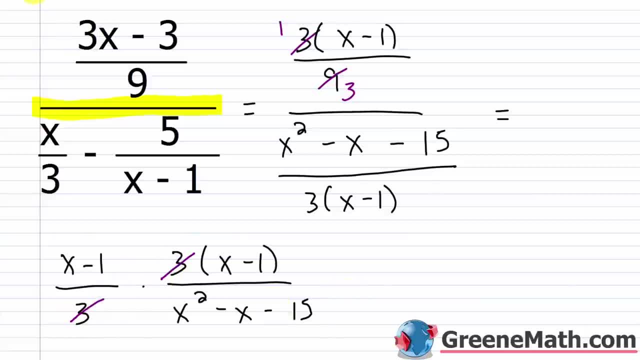 and then that's it so what i'm left with is x minus 1 that quantity times x minus 1 again we can say that's x minus 1 squared if we want 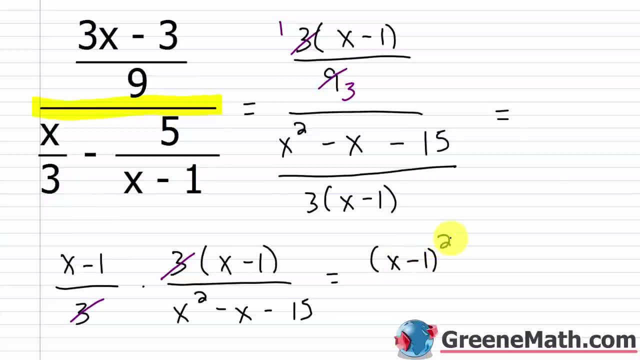 or your teacher might want you to go through and actually do the foil you know just to get some practice that's fine 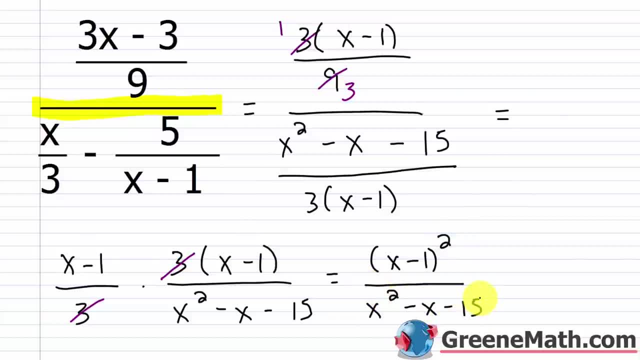 and then this is over x squared minus x minus 15 and just for the sake of completeness 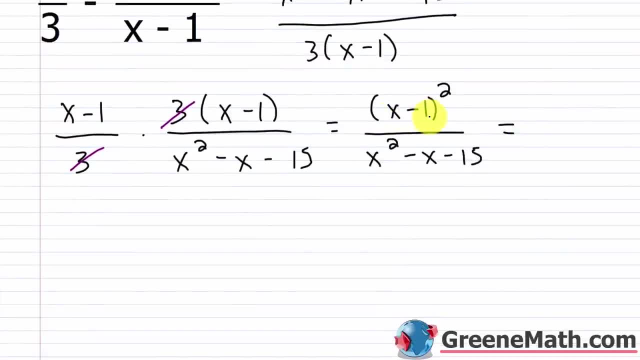 let's go ahead and do that if i have x minus 1 that quantity squared we can use our special products formula we know that would be x squared 2 times x times 1 so basically 2x and then plus this guy squared which would be 1 so x squared 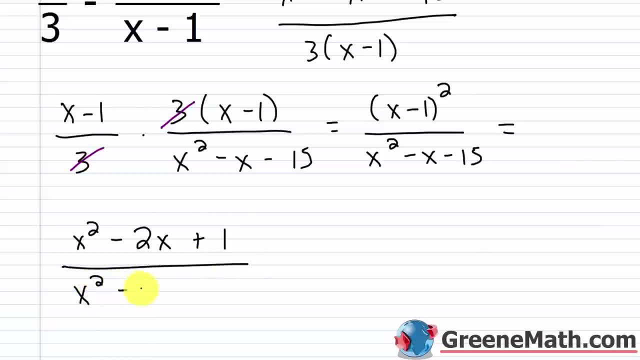 minus 2x plus 1 over x squared minus x minus 15 again a lot of people will rather leave it in factored form so that you can show your teacher hey there wasn't anything that i 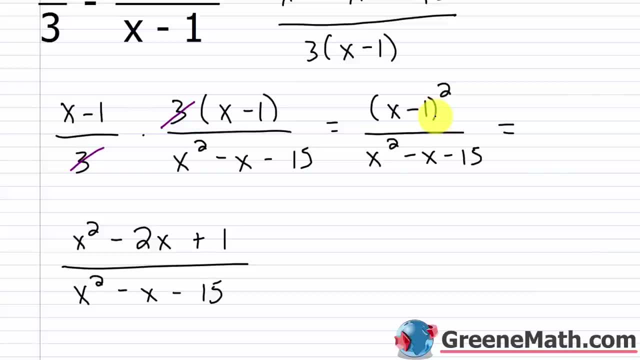 could cancel but again that kind of goes back and forth as far as what he or she may want you to do alright let's take a look at another one 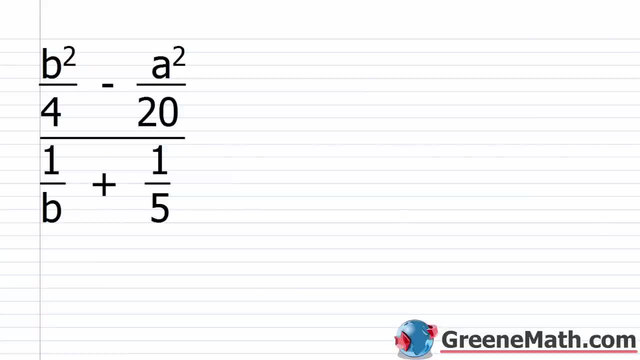 so i have b squared over 4 minus a squared over 20 and this is over 1 over b plus 1 over 5 so again i have my main division here right here 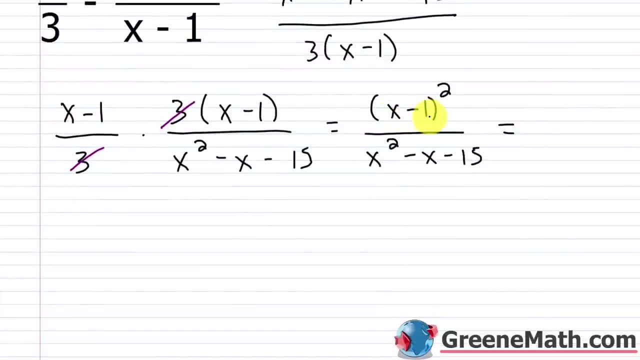 If I have x minus 1, that quantity squared, we can use our special products formula. We know that would be x squared minus 2 times x times 1.. So basically 2x And then plus this guy squared, which would be 1.. 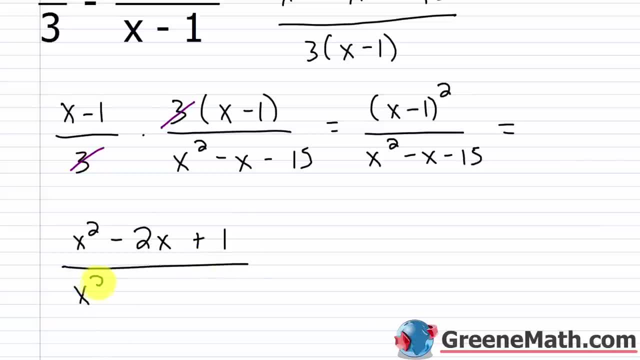 So x squared minus 2x plus 1 over x squared minus x minus 15.. Again, a lot of people will rather leave it in factored form so that you can show your teacher. hey, there wasn't anything that I could cancel. 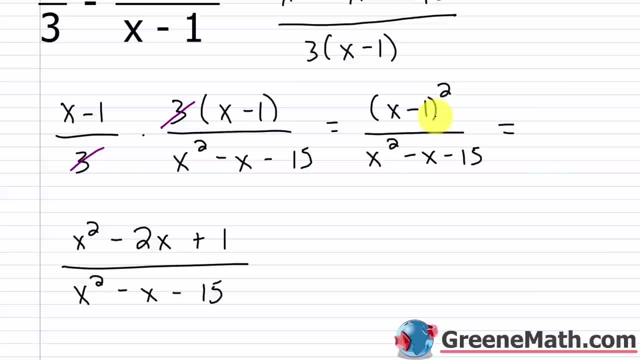 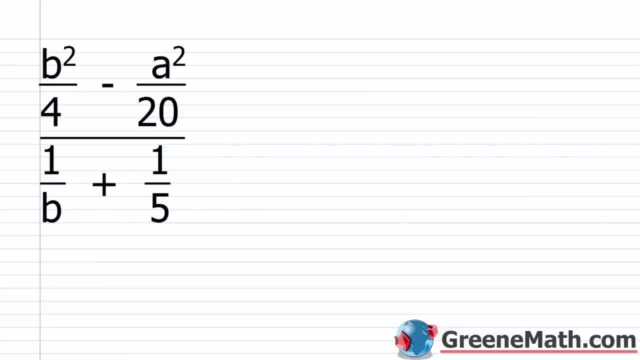 But again that kind of goes back and forth as far as what he or she may want you to do. All right, let's take a look at another one. So I have b squared over 4 minus a squared over 20. And this is over 1 over b plus 1 over 5.. 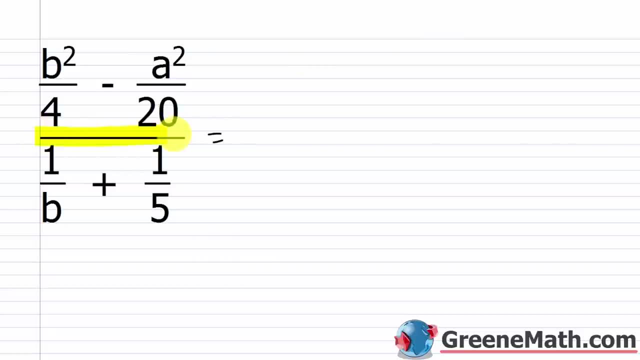 So again, I have my main division here, right here. So this is your numerator, This is your denominator right for the complex fraction. So if I look at this, I have b squared over 4 minus a squared over 20.. 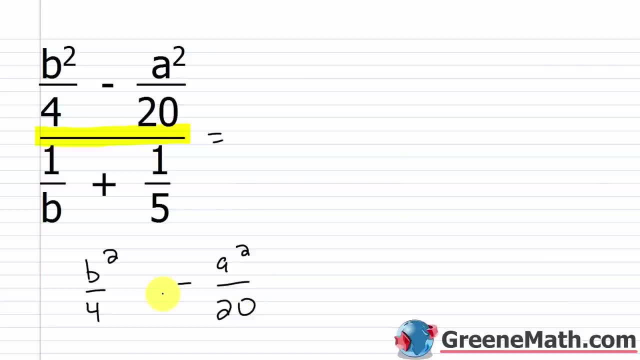 That's my numerator, So I'm going to start out by just simplifying that guy. Now the LCD here would be 20, right? 20 is going to factor into what? 2 times 2 times 5.. 4 factors into 2 times 2.. 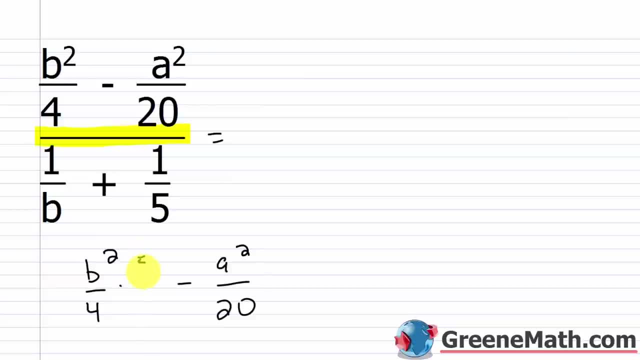 So essentially you need to multiply this by 5 over 5.. And then you'd have a common denominator. So this would be 5b squared minus a squared. I don't need to do anything over here Over that common denominator of 20.. 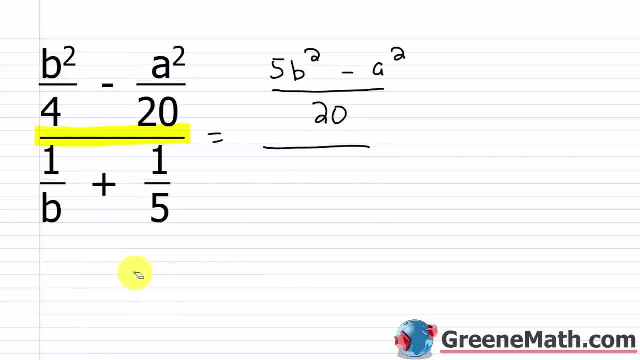 And then this is over. If I look at this guy right here, 1 over b plus 1 over 5, the LCD is going to be 5b 5, I'm not going to be able to factor and I can't do anything with b either. 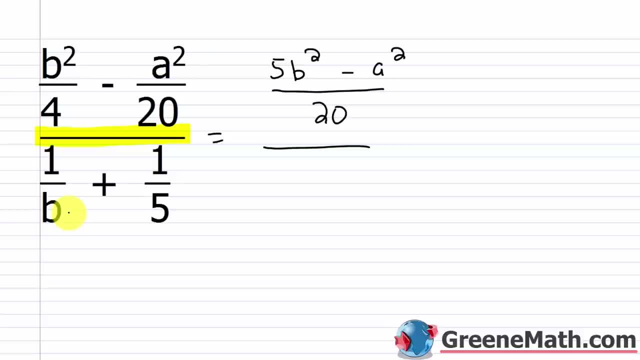 So I just have to multiply the two together, So 5 times b. So I'd multiply this guy 1 over b times 5 over 5.. And I'd multiply 1 over 5 times b over b. So 1 times 5 is 5, plus 1 times b is b. 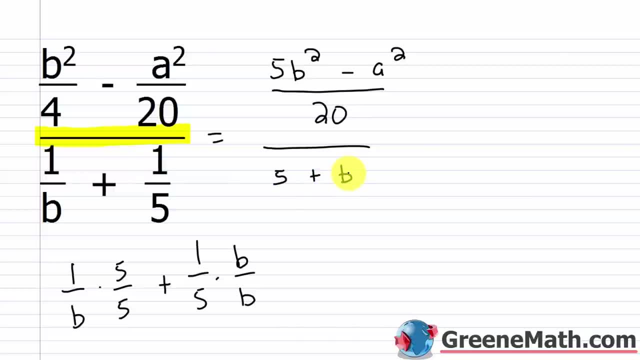 So you'd get 5 plus b, or you could put b plus 5, doesn't matter, 1 over 5b. Let me kind of reverse that and put b plus 5.. All right, so let's erase this real quick. 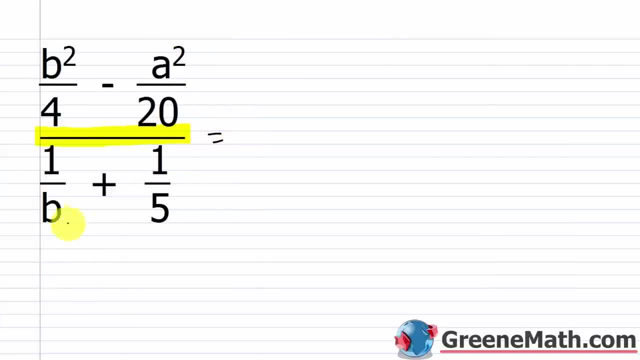 so this is your numerator this is your denominator right for the complex fraction so if i look at this i have b squared over 4 minus a squared over 20 that's my numerator so i'm going to start out by just simplifying that guy now the lcd here would be 20 right 20 is going to factor into what 2 times 2 times 5 4 factors into 2 times 2 so essentially you need to multiply this by 5 over 5 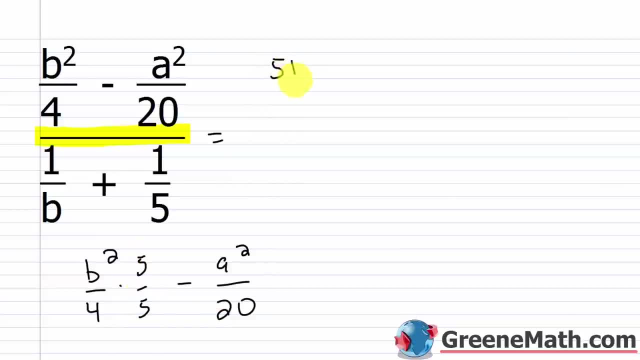 and then you'd have a common denominator so this would be 5 b squared minus a squared i don't need to do anything over here over that common denominator 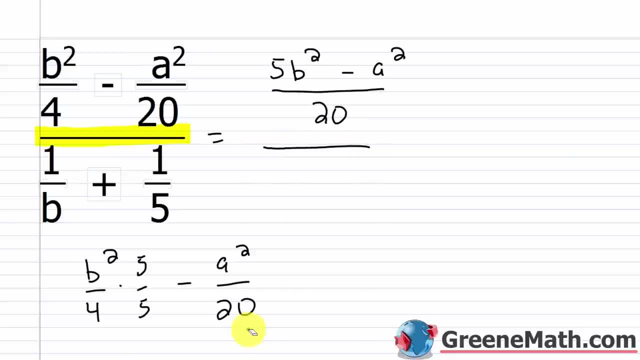 of 20 and then this is over if i look at this guy right here 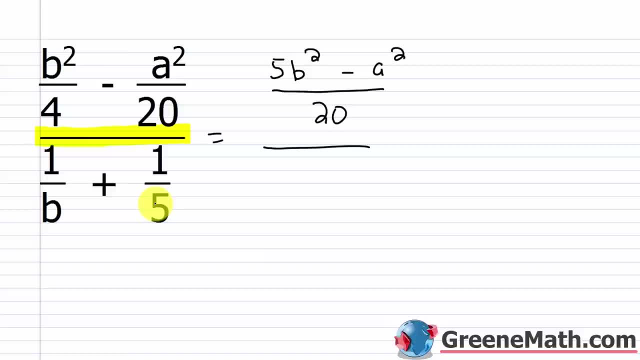 1 over b plus 1 over 5 the lcd is going to be 5 b 5 i'm not going to be able to factor and i can't do anything with b either so i just have to multiply the two together so 5 times b so i'd multiply this guy 1 over 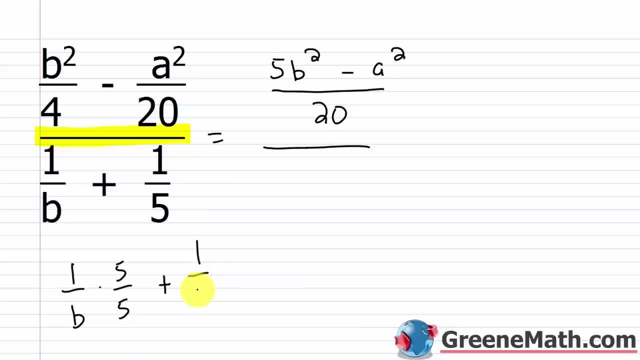 b times 5 over 5 and i'd multiply 1 over 5 times b over b so 1 times 5 is 5 plus 1 times b is b so you get 5 plus b or you could put b plus 5 doesn't matter over 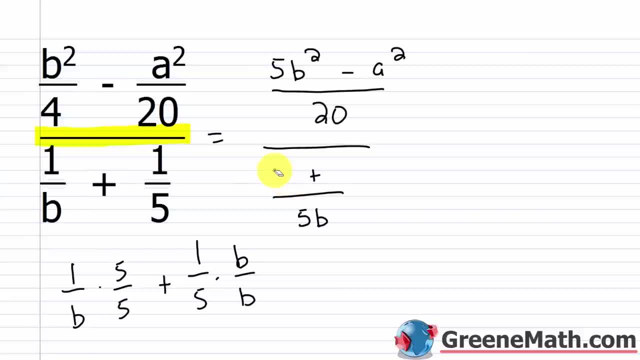 5b let me kind of reverse that and put b plus 5 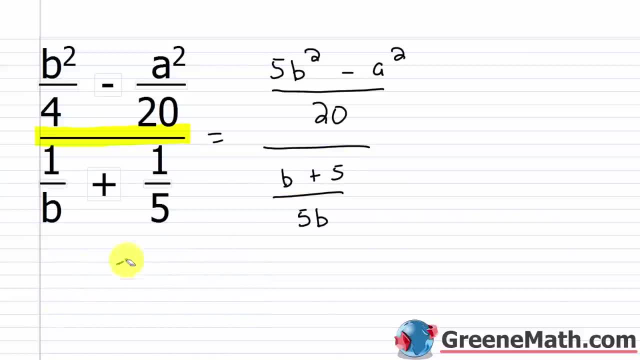 alright so let's erase this real quick 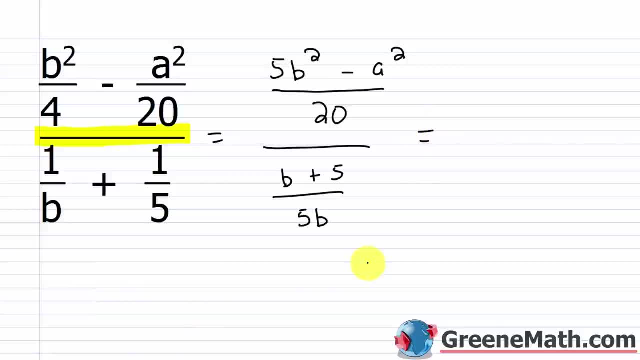 and again we're going to set up our multiplication so this top guy 5 b squared 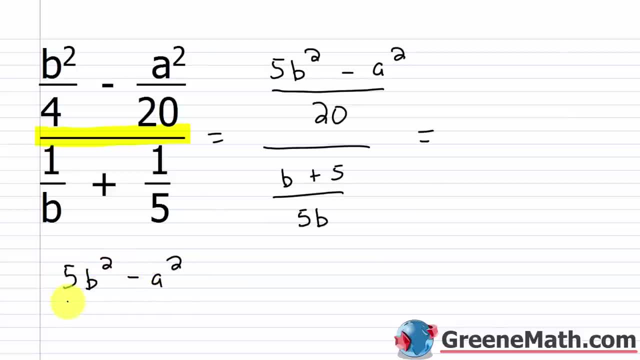 minus a squared over 20 is multiplied by the reciprocal of this guy i'm taking this and i'm dividing by this so the first one or the top one now stays unchanged we multiply by the reciprocal of the bottom one so this is 5b over b plus 5 now 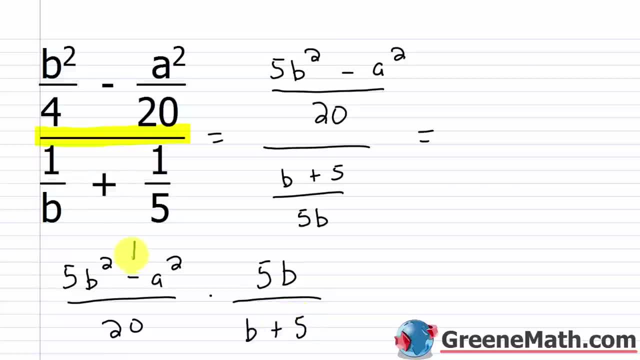 can i do anything to factor this guy right here if i didn't have that 5 there i could do 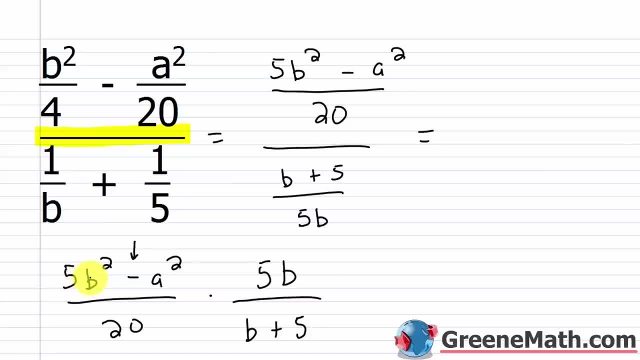 b plus a times b minus a be the difference of two squares 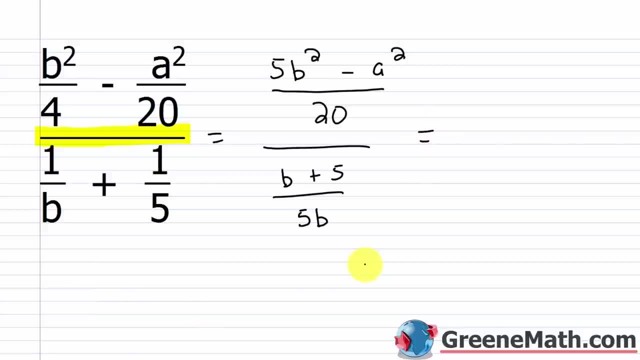 And again we're going to set up our multiplication. So this top guy, 5b, squared minus a squared over 20, is multiplied by the reciprocal of this guy. I'm taking this and I'm dividing by this, So the first one, or the top one, now stays unchanged. 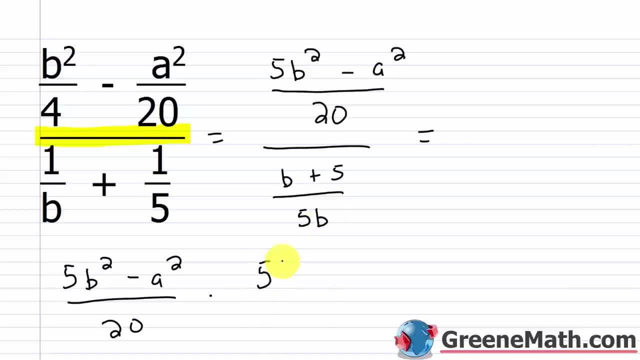 We multiply by the reciprocal of the bottom one, So this is 5b over b plus 5.. Now can I do anything to factor this guy right here? If I didn't have that 5 there, I could do b plus a times b minus a be the difference of two squares. 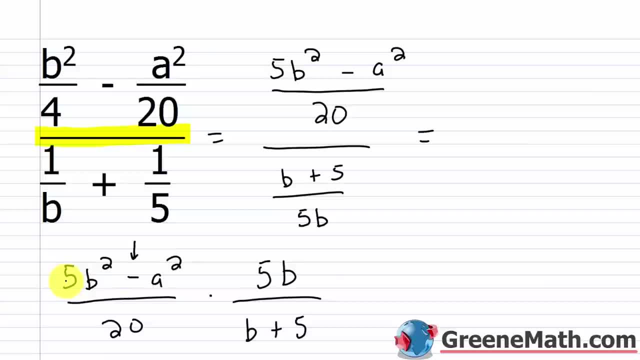 But I do have the 5 there, so that stops me from being able to do that. So there's not really anything I can pull out there. Now. over here I know I can do some things. I can do some canceling, because 5 and 20 have a common factor of 5.. 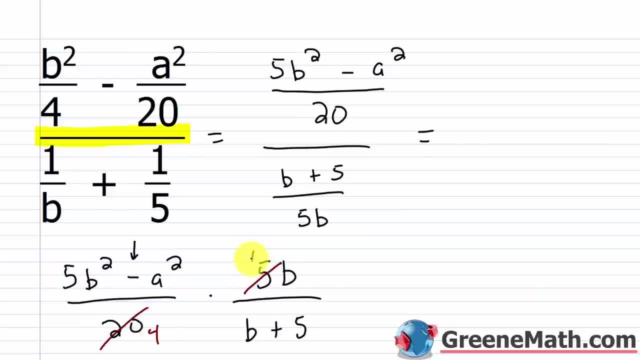 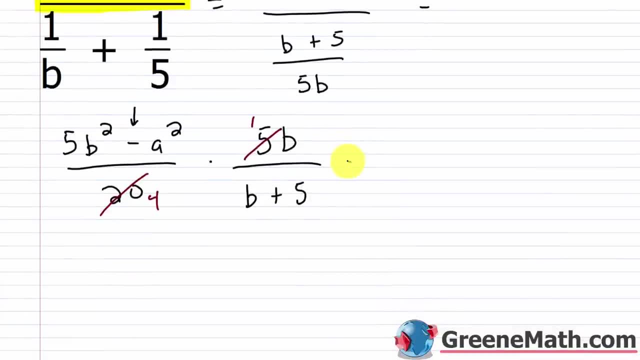 So this can cancel with this, And I'll put a 4 here and a 1 here And then I'm basically done. All I want to do now is just multiply. I can leave this in factor form and say, okay, this is b times the quantity 5b squared minus a squared. 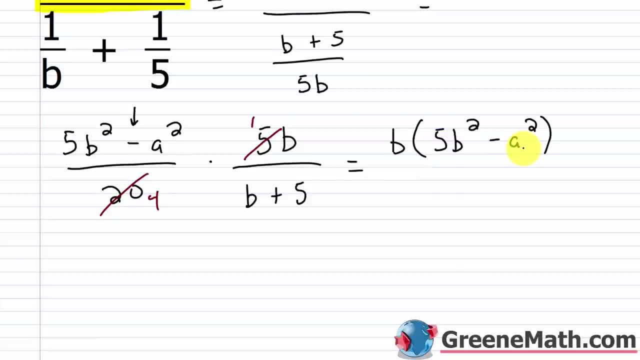 Or you can go through and use your distributive property. Again, that's going to be your personal preference or your teacher's preference. Again, this is over 4 times the quantity b plus 5. And again, if we want to go through, we can use our distributive property. just to show both answers. 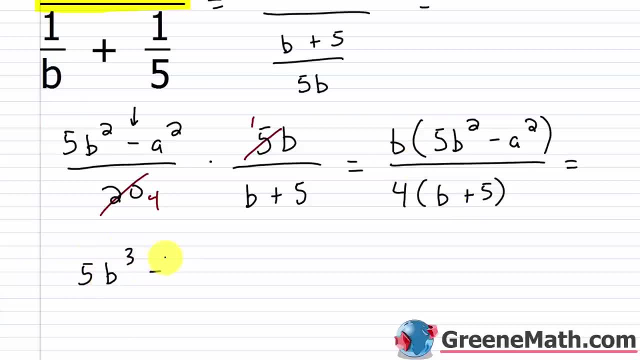 b times 5b squared is 5b cubed. Then minus b times a squared is a squared b. This is over 4 times b is 4b And then plus 4 times 5 is 20.. So we get 5b cubed minus a squared b over 4b plus 20.. 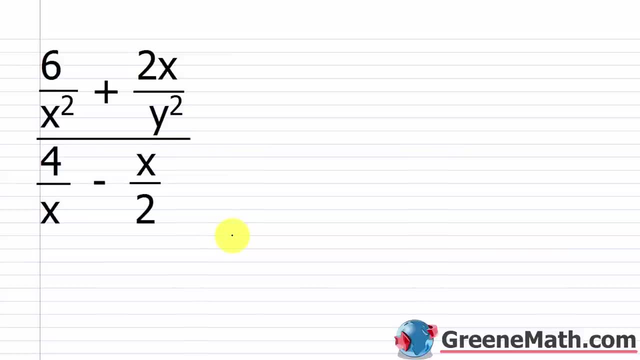 All right, let's take a look at one final problem, kind of using this method, And then we'll kind of look at the LCD method to wrap up the lesson. So if I look at 6 over x squared plus 2x over y squared, then this is over 4 over x, minus x over 2.. 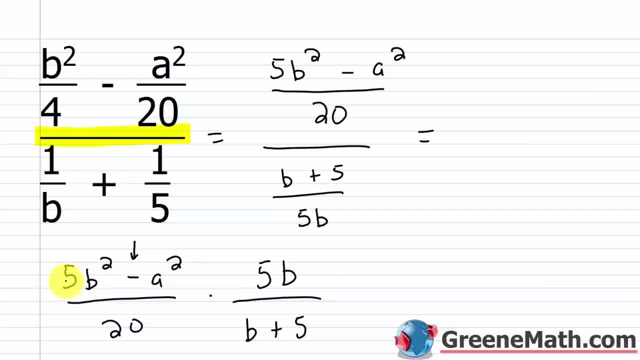 but i do have the 5 there so that stops me from being able to do that so there's not really anything i can pull out there 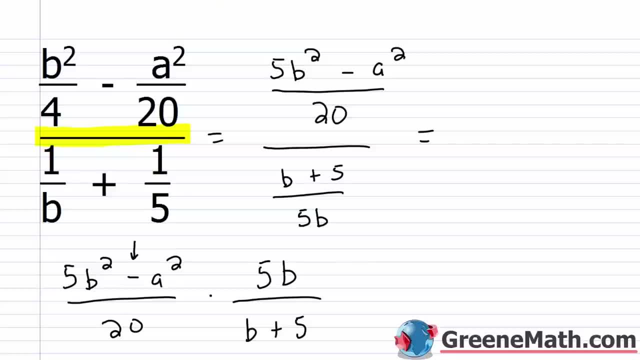 now over here i know i can do some canceling 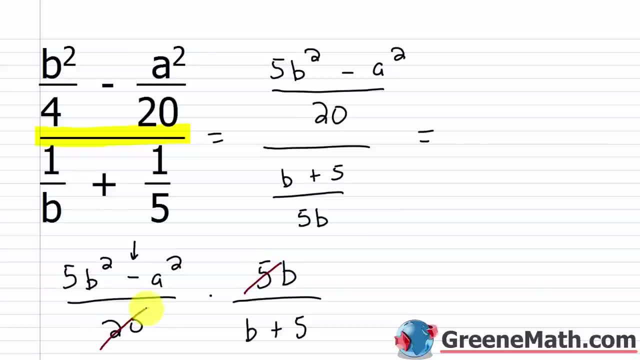 because 5 and 20 have a common factor of 5 so this can cancel with this and i'll put a 4 here and a 1 here 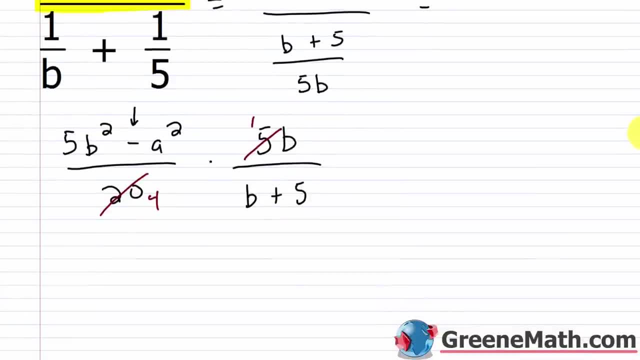 and then i'm basically done all i want to do now is just multiply 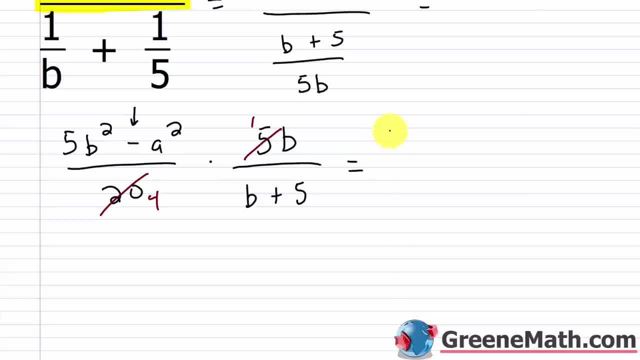 i can leave this in factor form and say this is b times 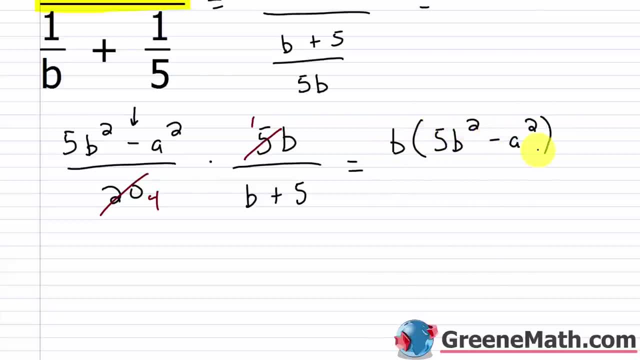 the quantity 5 b squared minus a squared or you can go through and use your distributive property again that's going to be your personal preference 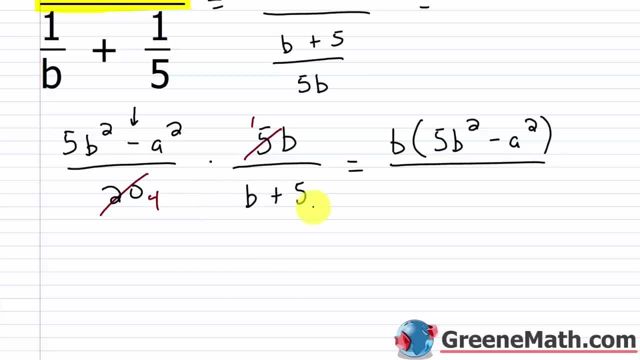 or your teachers preference again this is over 4 times the quantity b plus 5 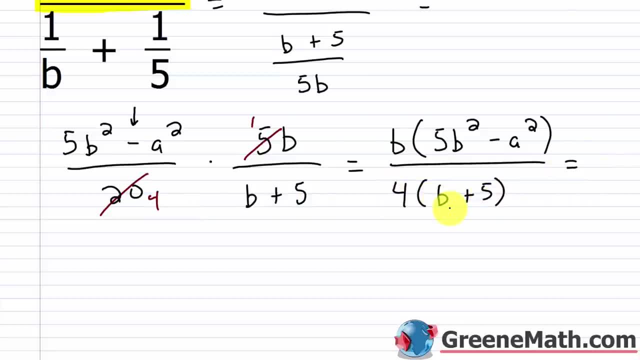 and again if we want to go through we can use our distributive property just to show both answers b times 5 b squared is 5 b cubed 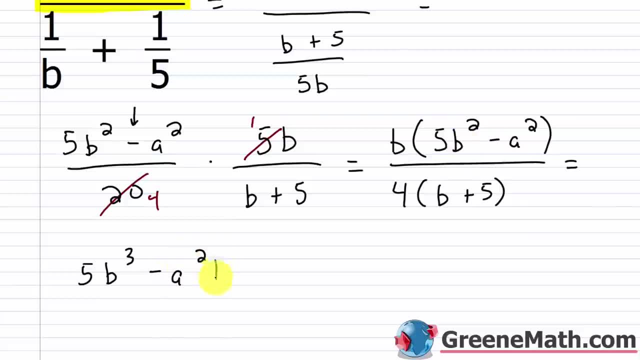 then minus b times a squared is a squared b this is over 4 times b is 4 b and then plus 4 times 5 is 20 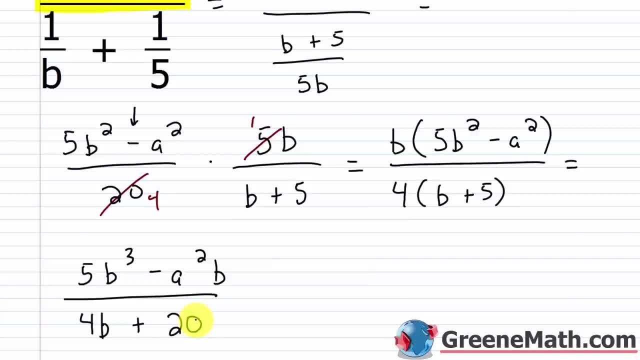 so we get 5 b cubed minus a squared b over 4 b plus 20 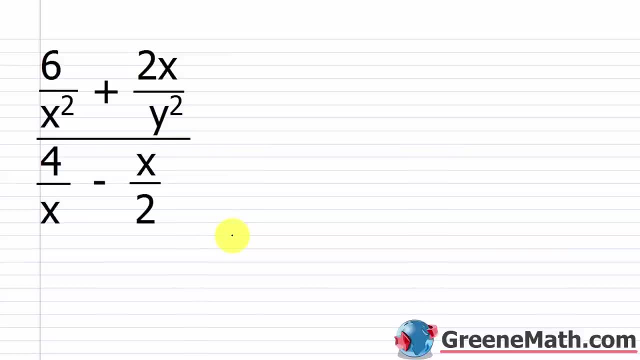 alright let's take a look at one final problem kind of using this method and then we'll kind of look at the lcd method to wrap up the lesson 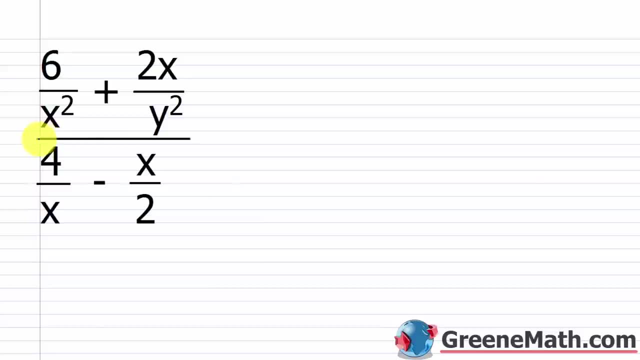 so if i look at 6 over x squared plus 2x over y squared over 4 over x minus x over 2 so again this is the numerator for the complex fraction this is the denominator for the complex fraction this part right here is your main division 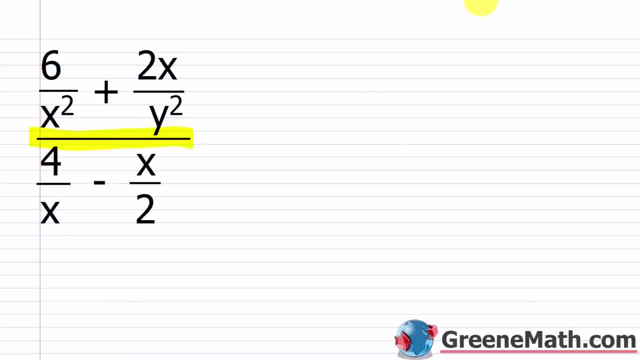 your main division so for the numerator if i have something like 6 over x squared plus 2x over y squared the lcd would just be x squared times y squared nothing else we can do there so i'd multiply this by y squared over y squared multiply this by x squared over x squared and the numerator would end up being 6y squared plus 2x cubed over x squared y squared ok 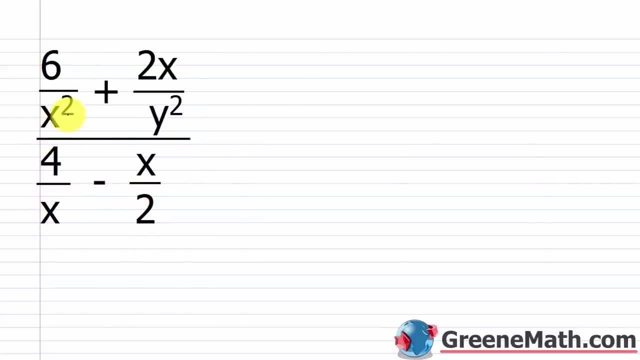 So again, this is the numerator for the complex fraction, This is the denominator for the complex fraction. This part right here is your main division. Okay, your main division. So for the numerator, I have something like 6 over x, squared plus 2x over 2.. 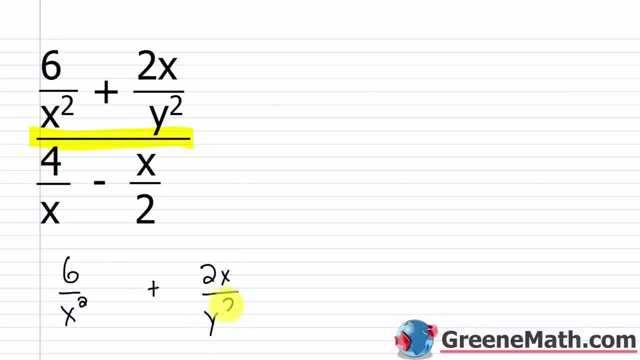 Plus 2x over y squared, The LCD would just be x squared times y squared, Nothing else we can do there. So I'd multiply this by y squared over y squared. I'd multiply this by x squared over x squared, And the numerator would end up being 6y squared plus 2x cubed over x squared, y squared. 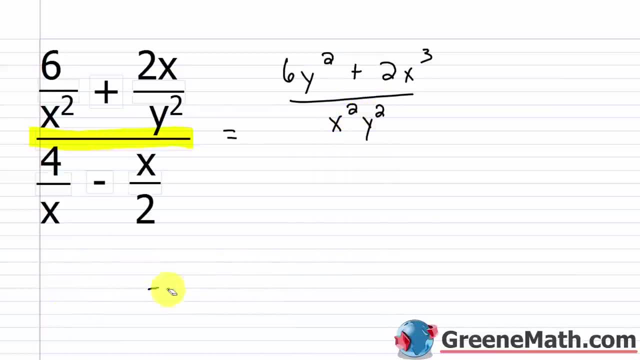 Okay, Now for the denominator down here. What do we have? 4 over x minus x over 2.. So the LCD here would be 2x. So 4 over x times 2 over 2 minus x over 2 times x over x. 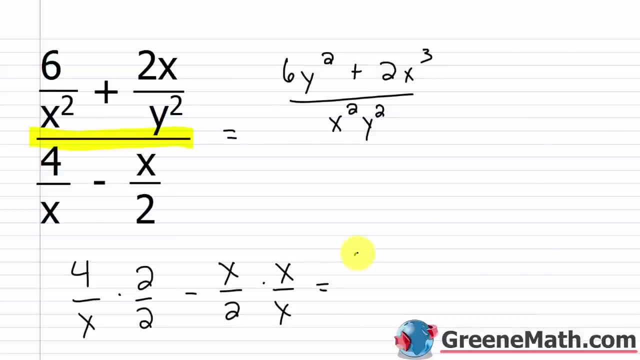 So this would be equal to 8 over 2x, minus x squared over 2x. So I'll write this over: 8 minus x, squared Again over 2x. So let me erase all this real quick. So we're going to set this up as a multiplication. 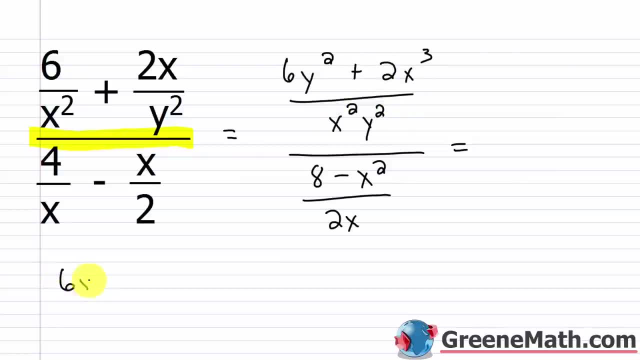 So this top part right here, 6y squared plus 2x cubed over x squared, y squared will be multiplied by the reciprocal of this guy, which is 2x over 8 minus x squared. Now what can I do to simplify? 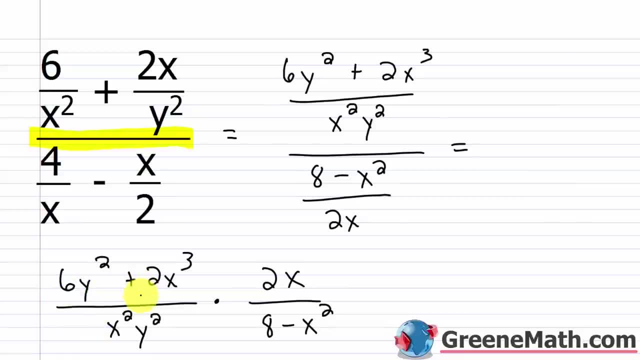 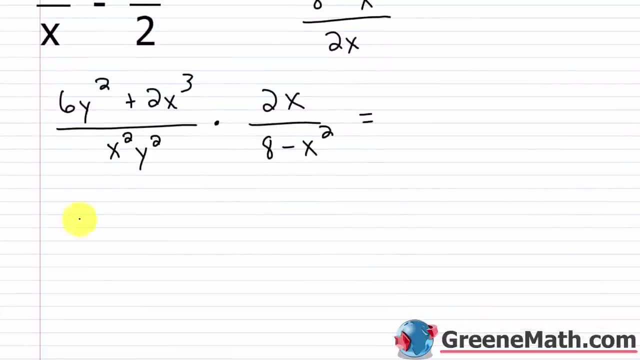 I noticed that I could pull out a 2 from here, But it's not going to do me any good, But I'm just going to go ahead and factor it anyway. Let me kind of scroll down a little bit. So if I pulled out a 2 from here, I'd have 3y squared plus x cubed. 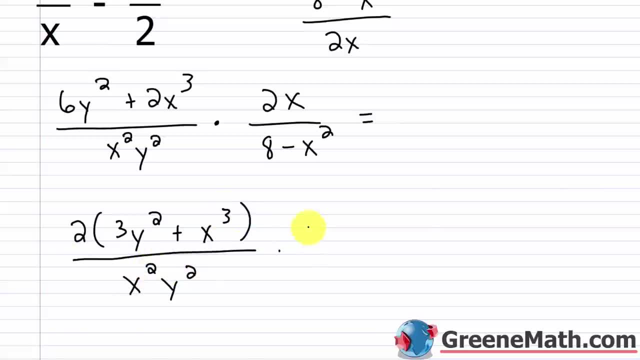 This is over again. x squared, y squared times 2x over 8 minus x squared. Nothing I can cancel between numerator and denominator here. Nothing I can cancel between the numerator and denominator here. The only thing I can cancel is one factor of x. 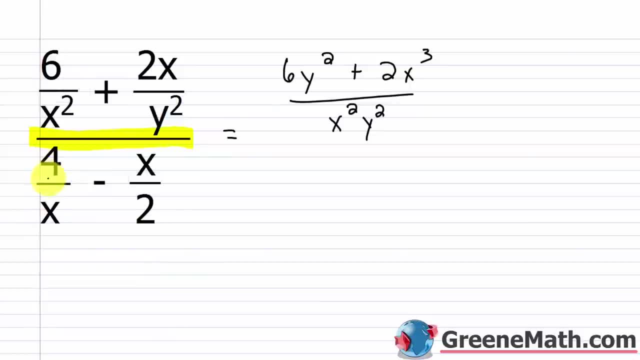 now for the denominator down here what do we have 4 over x minus x over 2 so the lcd here would be 2x so 4 over x times 2 over 2 minus x over 2 times x over x so this would be equal to 8 over 2x minus x squared over 2x so i'll write this over 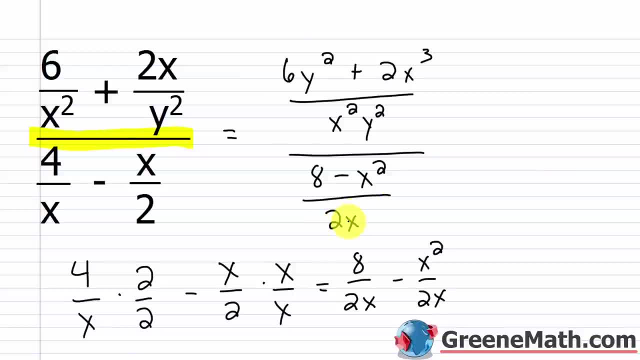 8 minus x squared again over 2x so let me erase all this real quick 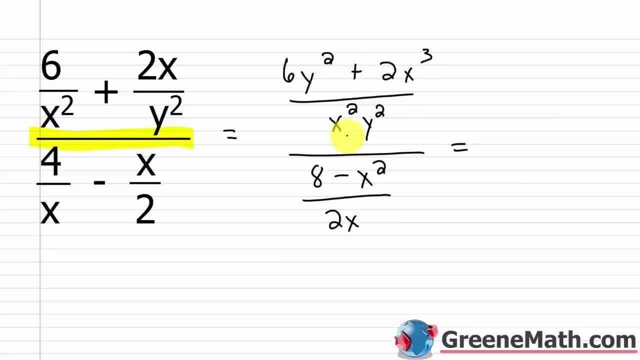 so we're going to set this up as a multiplication so this top part right here 6y squared plus 2x cubed over x squared y squared will be multiplied by the reciprocal of this guy 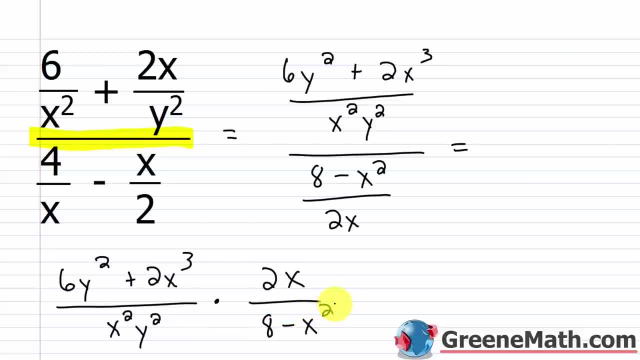 which is 2x over 8 minus x squared now what can i do to simplify 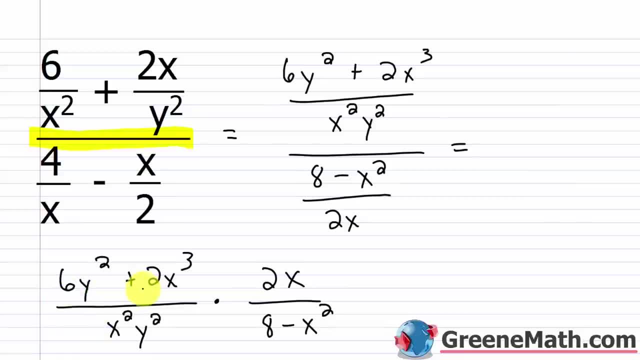 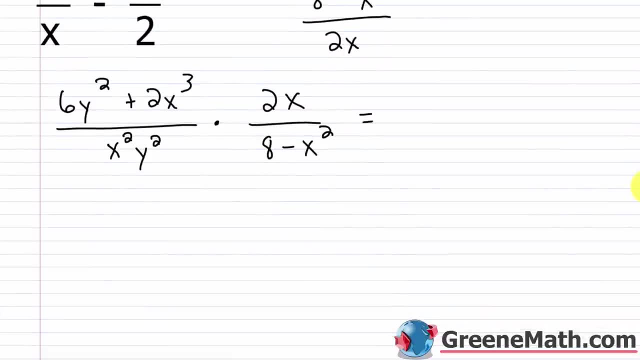 i noticed that i could pull out a 2 from here but it's not going to do me any good but i'm just going to go ahead and factor it anyway let me kind of scroll down a little bit so if i pulled out a 2 from here i'd have 3y squared plus x cubed this is over again squared y squared times 2x over 8 minus x squared nothing i can cancel between numerator and denominator here 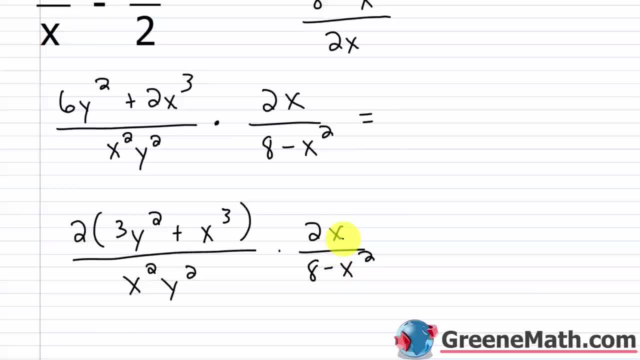 nothing i can cancel between the numerator and denominator here 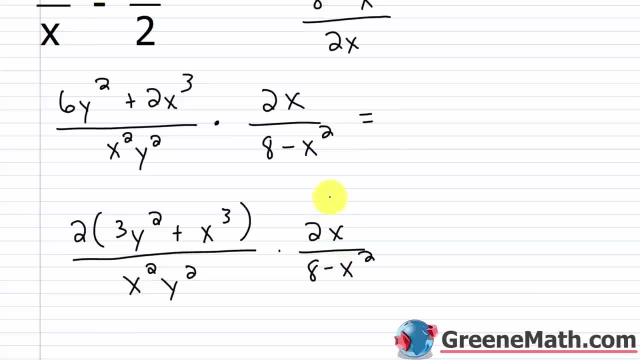 the only thing i can cancel is one factor of x 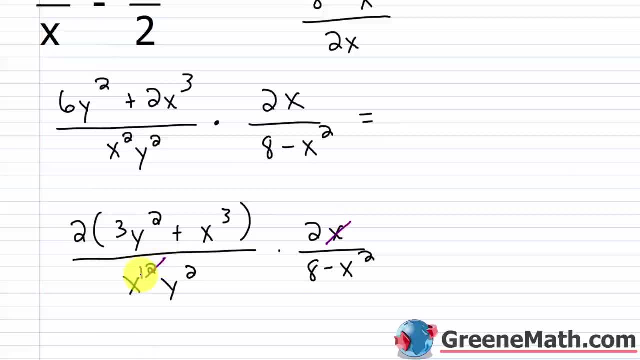 here with here this would be x to the first power that's it other than that i'm pretty much done 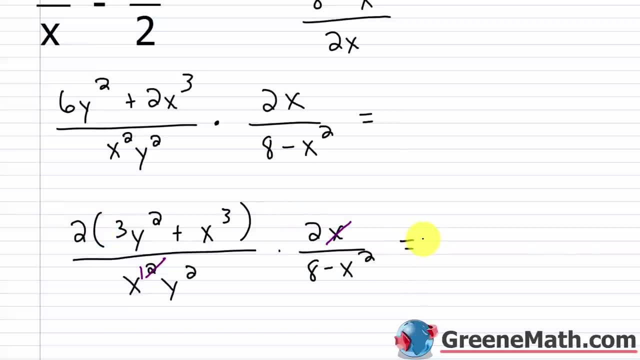 now i multiply 2 times 2 i would get 4 so i can put this as 4 times that quantity 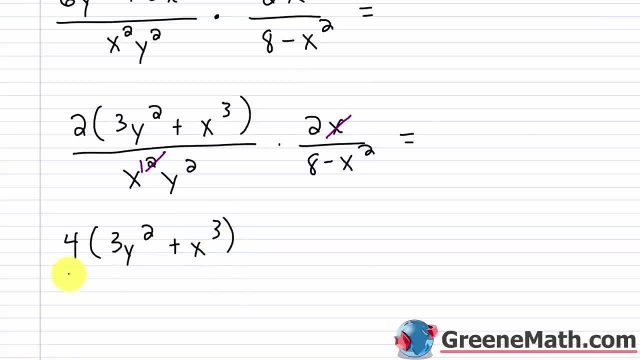 4 times 3y squared plus x cubed and then over then i would have xy squared times the quantity 8 minus x squared 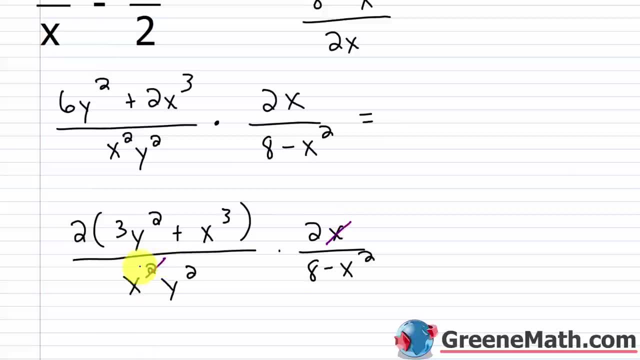 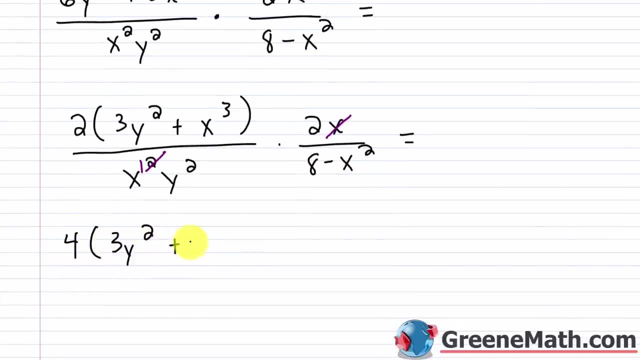 One factor of x here with here This would be x to the first power. That's it. Other than that, I'm pretty much done Now. I multiply 2 times 2, I would get 4.. So I can put this as 4 times that quantity, 3y squared plus x cubed. 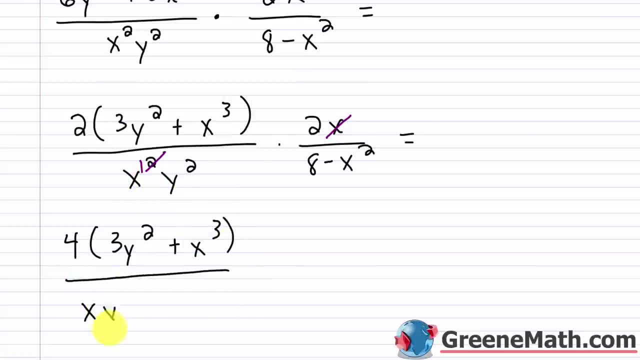 And then over then I would have xy squared times the quantity 8 minus x squared. Now Your teacher may let you leave it in this format. In most cases that's what I would do, But she might also want you to get a little practice and use your distributive property. 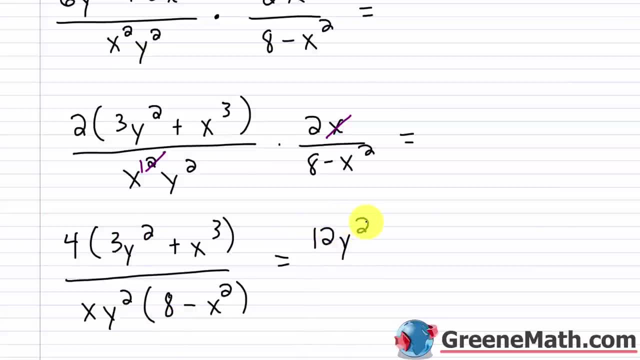 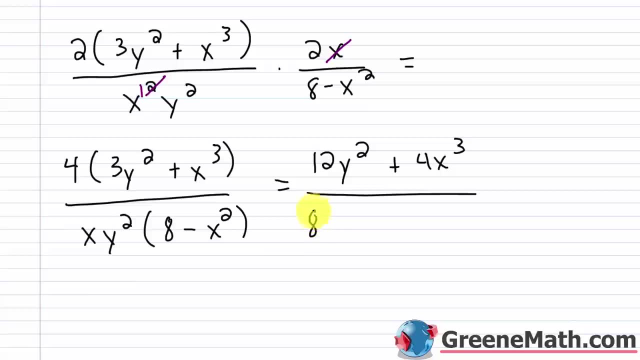 So 4 times 3y squared is 12y squared. Then 4 times x cubed is plus 4x cubed, And then over you have xy squared times 8. That's 8xy squared. And then you have xy squared times negative x squared. 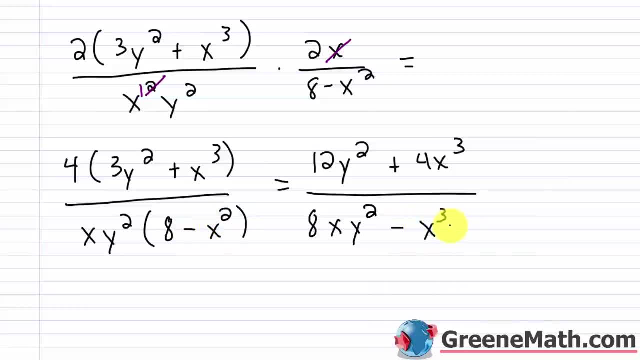 That is minus x cubed, y squared. And for some of you you'll want to write this where 4x cubed is in the front here. So you can do that. You can switch the order and say: okay, this is 4x cubed plus 12y squared over switch. 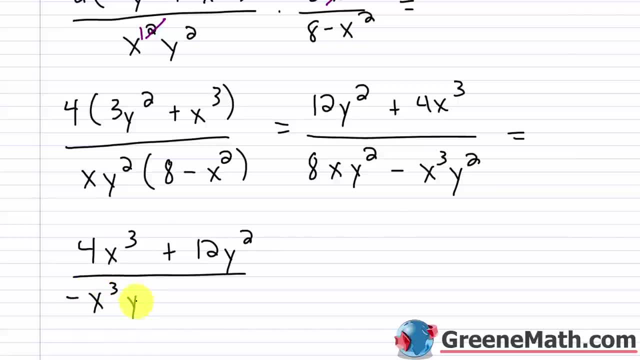 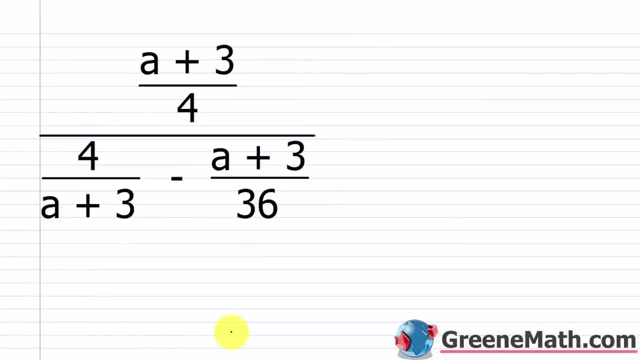 the order here: negative: x cubed, y squared plus 8xy squared. All right, Let's take a look at a few that deal with the LCD method now. I think for the majority of you you will prefer to use this method because it's a lot. 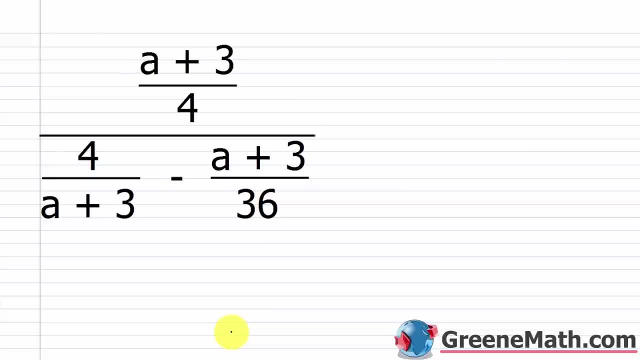 quicker to use in most scenarios. Now, with that being said, it's a little bit challenging to kind of understand what you need to actually do when you first start utilizing this method. But just like anything else, if you practice this enough, you'll get really good at it. 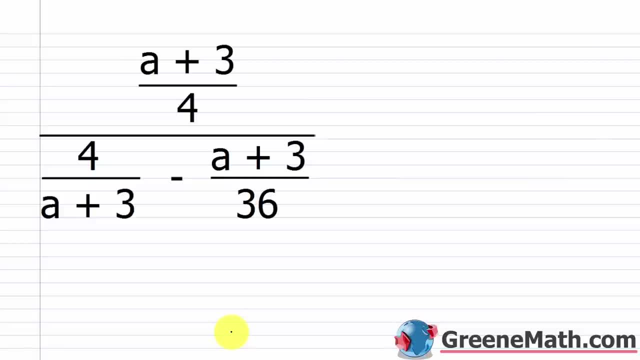 And again, you'll prefer this method because generally it's a lot quicker. All right, So let's take a look at a plus 3 over 4 and then over 4 over a plus 3, and then minus a plus 3 over 36.. 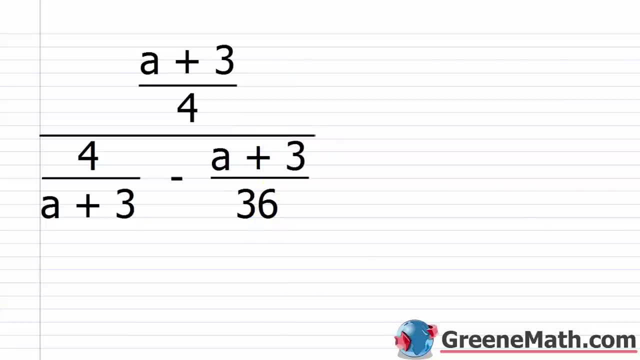 So recall that the complex fraction has a plus 3 over 4.. It has a numerator, And let me kind of label this real quick. This is the numerator And then it also has a denominator. So this is your denominator And then recall that this is your main fraction, bar right here. 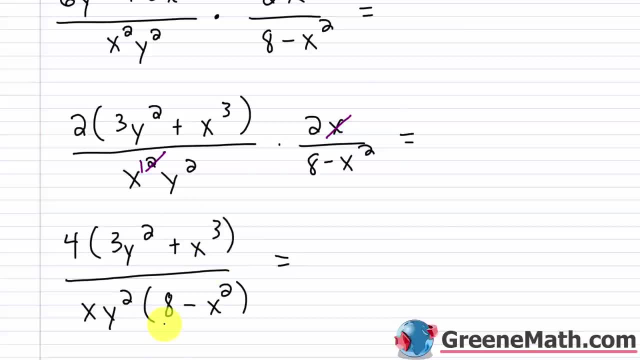 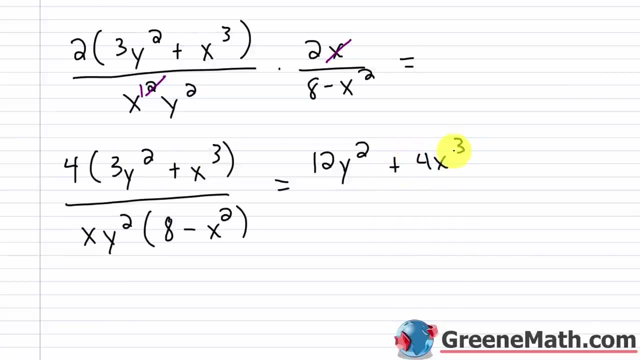 now your teacher may let you leave it in this format in most cases that's what i would do but she might also want you to get a little practice and use your distributive property so 4 times 3y squared is 12y squared then 4 times x cubed is plus 4x cubed over you have xy squared times 8 that's 8xy squared and then you have xy squared times negative x squared that is minus x cubed 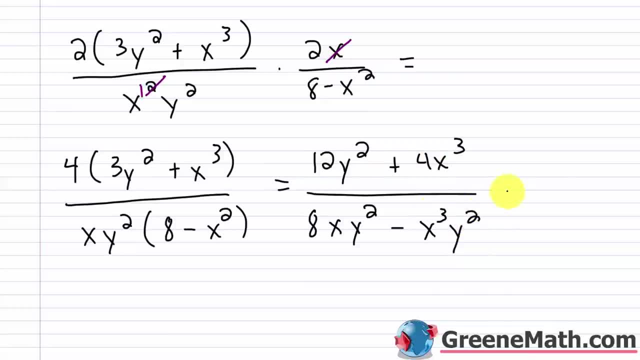 y squared and for some of you you'll want to write this where 4x cubed is in the front here so you can do that you can switch the order and say okay this is 4x cubed plus 12y squared over switch the order 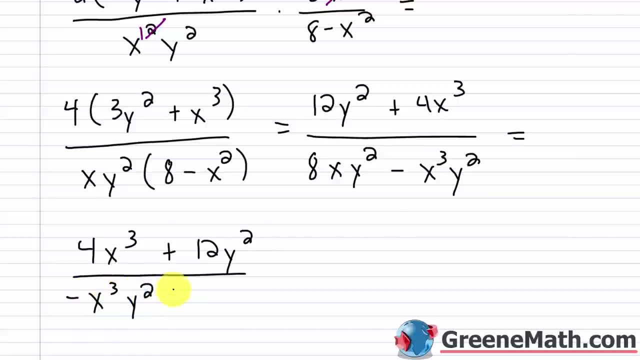 here negative x cubed y squared plus 8xy squared all right let's take a look 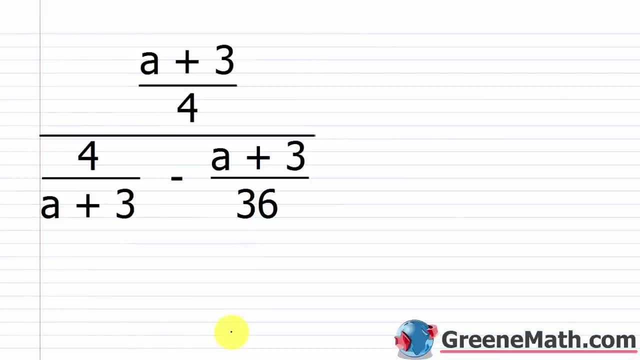 at a few that deal with the lcd method now i think for the majority of you you will prefer to use this method because it's a lot quicker 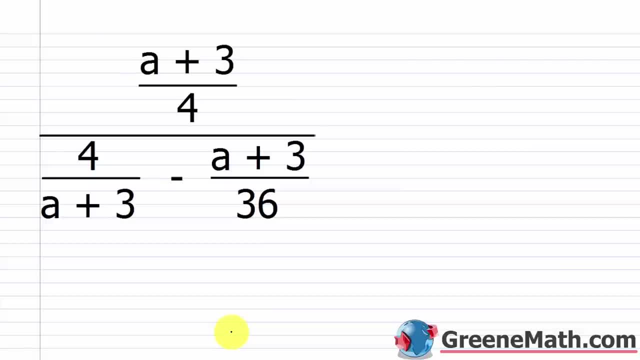 to use in most scenarios now with that being said it's a little bit challenging to kind of understand what you need to actually do when you first start utilizing this method but just like anything else if you practice this enough you'll get really good at it and again you'll prefer this method 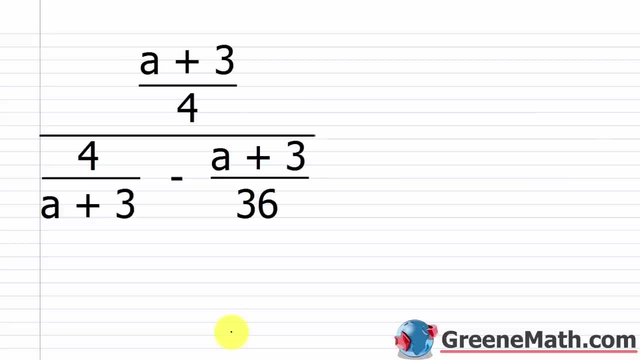 because generally it's a lot quicker all right so let's take a look at a plus 3 over 4 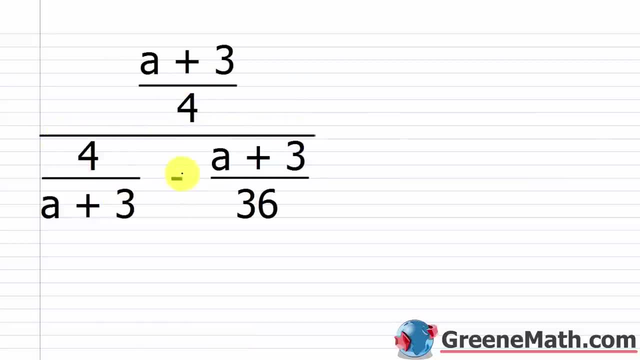 and then over 4 over a plus 3 and then minus a plus 3 over 36 so recall that the complex fraction 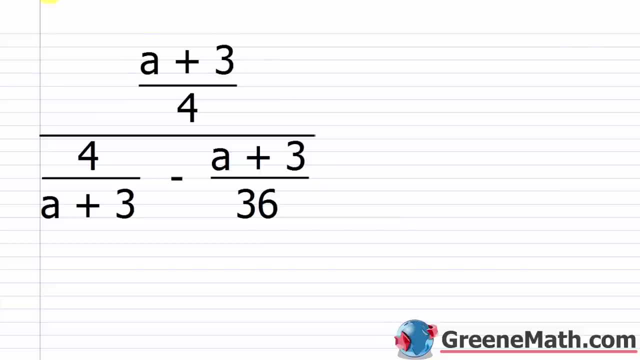 has a numerator and let me kind of let me kind of label this real quick this is the numerator 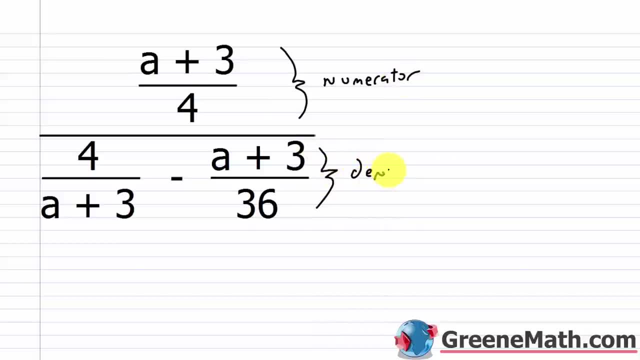 and then it also has a denominator so this is your denominator 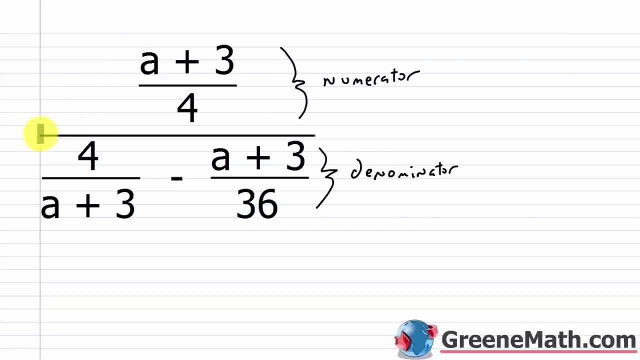 and then recall that this is your main fraction bar right here so let me just highlight that this is the main fraction bar or main division again as i've said before when you have a fraction it's the numerator divided by the denominator so 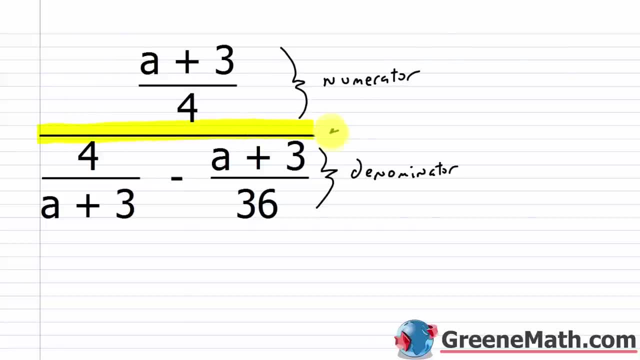 So let me just highlight that This is the main fraction, bar or main division. Again, as I've said before, when you have a fraction, it's the numerator divided by the denominator. So we have our numerator divided by our denominator. So, in the method that we've been using up to this point, I would take this numerator. 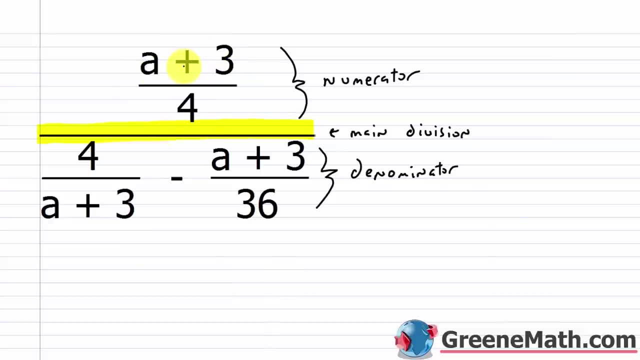 And once it's simplified- in this case it already is- I would multiply it by the reciprocal of this simplified denominator. I'm just basically performing a division. In the case of the method we're going to use right now, we're going to kind of speed up. 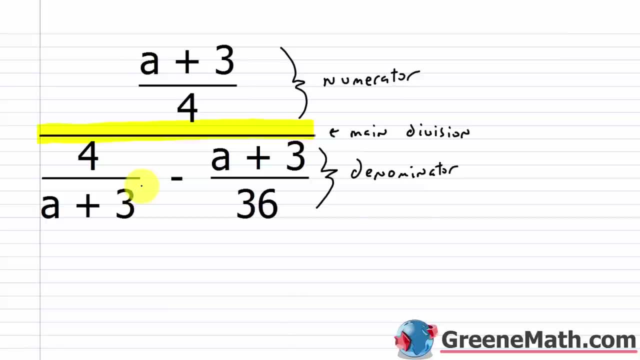 the process a little bit And we're basically going to clear all these denominators. The way we're going to do that is we're going to multiply by the numerator Of the complex fraction and the denominator of the complex fraction by the LCD for all. 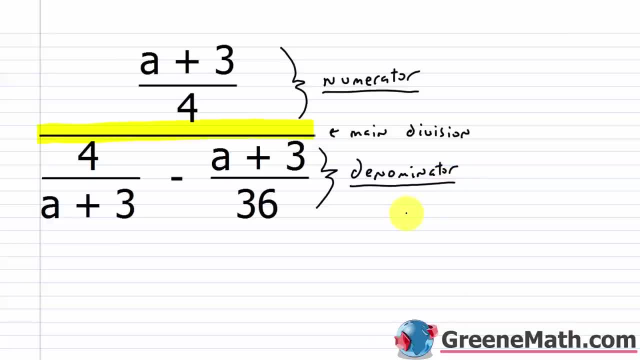 the fractions that are involved in the complex fraction. So if I were to look at each denominator individually for all the fractions I have involved, I have this denominator that's 4,, a denominator that is a plus 3, and a denominator that's 36.. 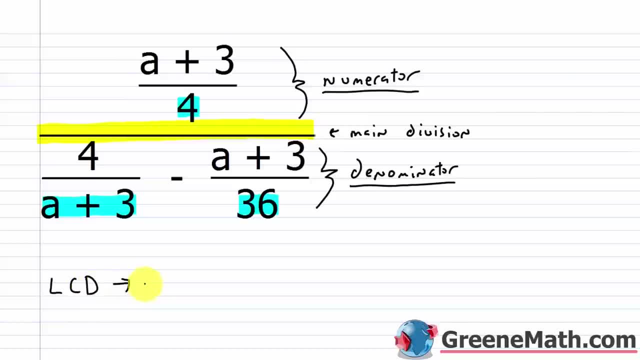 So to get the LCD, I just think about the LCM, the least common multiple of these three values. Again, I'm thinking about 4,, I'm thinking about 36, and I'm thinking about the quantity a plus 3.. 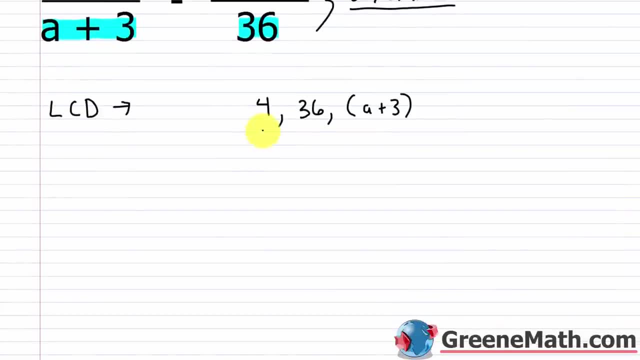 Well, this one's pretty easy, because if I think about 4, it's what It's going to factor into 2 times 2.. 36 has 4 as a factor, right? 36 I could factor into 4 times 9,, right. 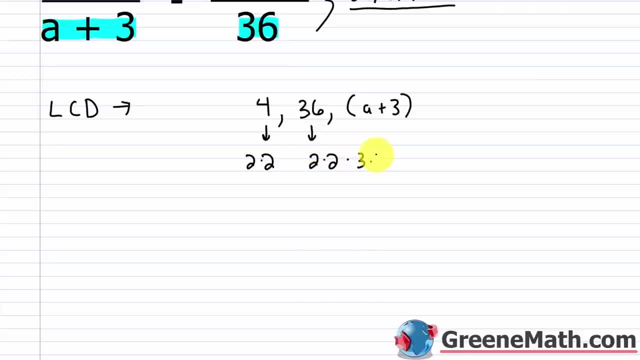 4 again is 2 times 2. And 9 is 3 times 3.. So for the number part of this guy I would basically have 2 times 2.. Times 3 times 3, or just 36.. 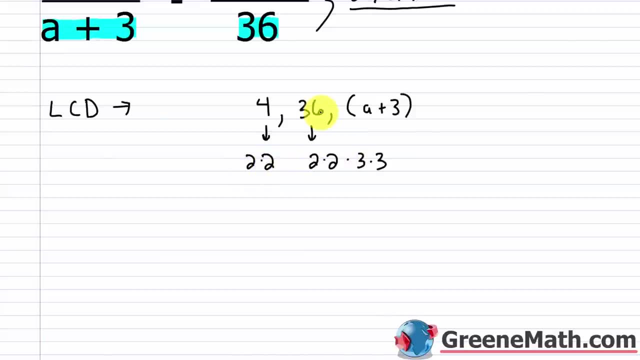 Right, if 4 is a factor of 36, then 36 is going to be the number part, Then times, I have that a plus 3, that quantity, So this over here, this a plus 3.. So once we've found the LCD, which is usually the most challenging part of this for students, 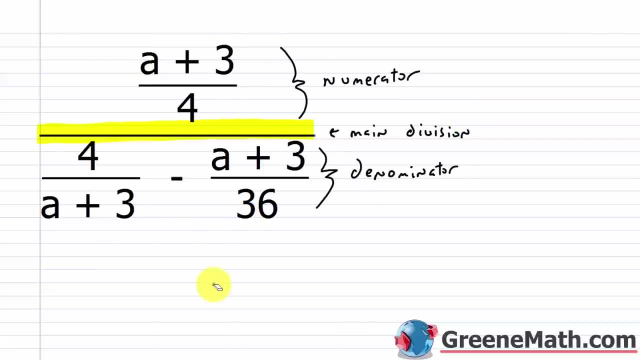 we have our numerator divided by our denominator so in the method that we've been using up to this point i would take this numerator and once it's simplified in this case it already is i would multiply it by the reciprocal of this simplified denominator right i'm just basically performing a division in the case of the method we're going to use right now we're going to kind of speed up the process a little bit and we're basically going to clear all these denominators the way we're going to do that is we're going to multiply the numerator of the complex fraction 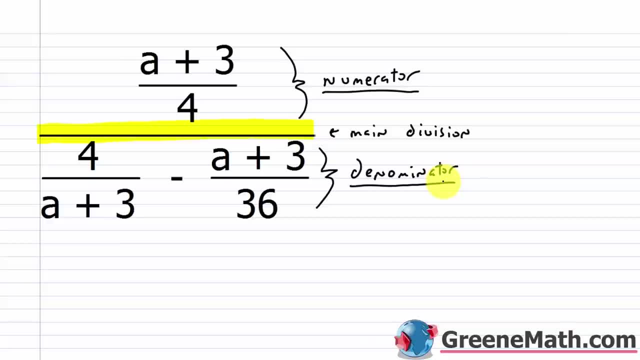 and the denominator of the complex fraction by the lcd for all the fractions that are involved in the complex fraction so if i were to look at each denominator individually for all the fractions i have involved i have this denominator that's four a denominator that is a plus three and a denominator that's thirty six so to get the lcd i just think about the lcm the least common multiple of these three values again i'm thinking about four i'm thinking about thirty six 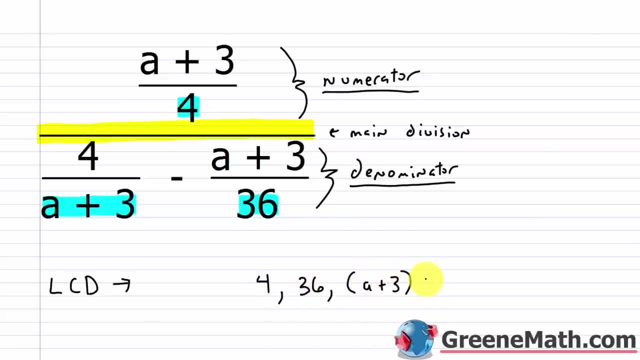 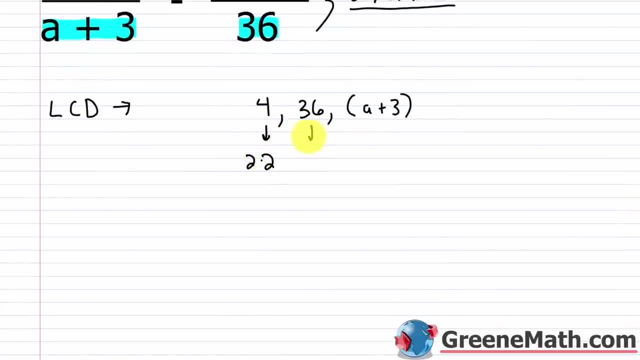 and i'm thinking about the quantity a plus three well this one's pretty easy because if i think about four it's what it's gonna factor into two times two thirty six has four as a factor right thirty six i could factor into four times nine right four again is two times two and nine is three times three so for the number part of this guy i would basically have two times two times three times three or just thirty six right if four is a factor of thirty six 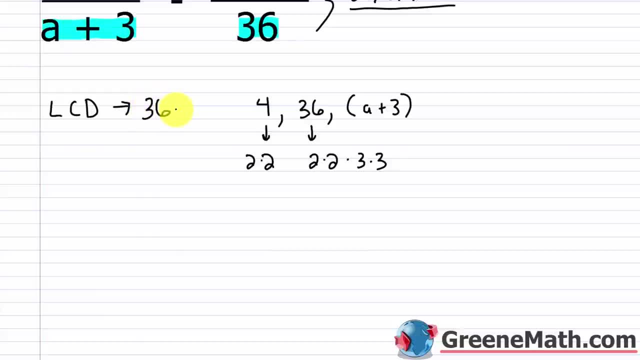 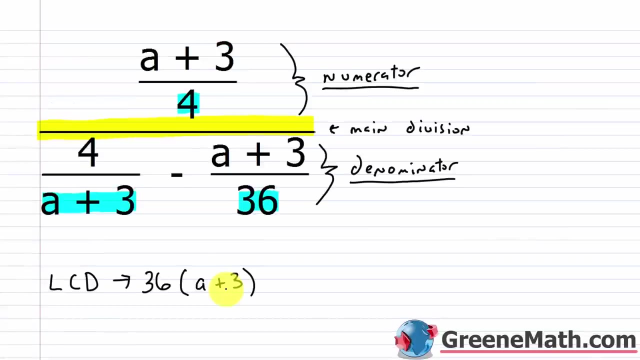 then thirty six is going to be the number part then times i have that a plus three that quantity so this over here this a plus three so once we've found the lcd which is usually the most challenging part of this for students because they're not fully up to speed on that yet we want to multiply the numerator and denominator of the complex fraction by that lcd and again your denominators for each fraction are going to disappear so let me erase this real quick we know what the numerator and denominator 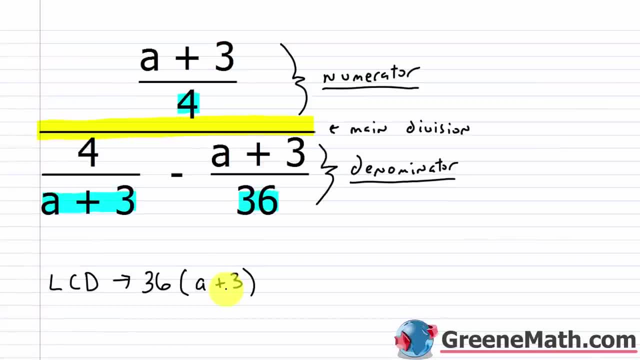 because they're not fully up to speed on that yet. we want to multiply the numerator and denominator of the complex fraction by that LCD And again your denominators for each fraction are going to disappear. So let me erase this real quick. We know what the numerator and denominator is at this point. 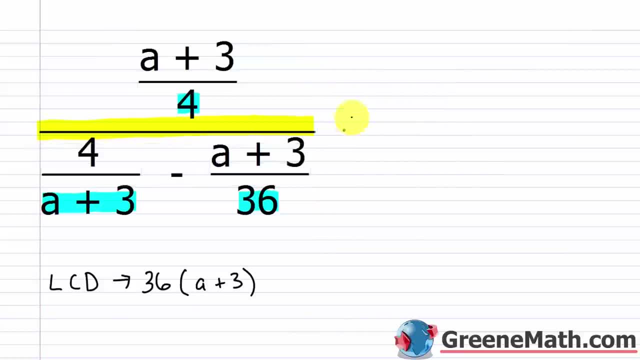 And I'm going to put a multiplication symbol right here And I'm going to be multiplying the numerator of the complex fraction by this: 36 times the quantity a plus 3.. And I'm going to do the same thing to the denominator. And why is this legal? before we move forward, 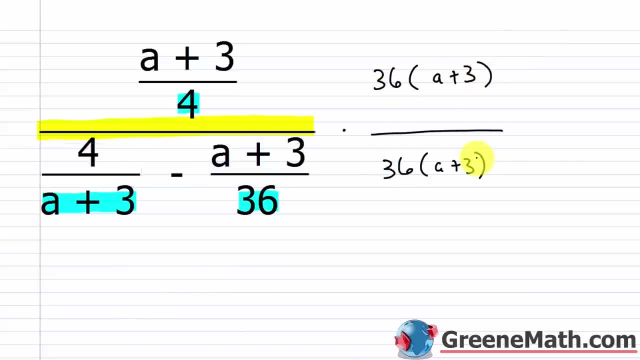 Again, this quantity over this quantity is equal to 1.. Right, So the integral value over itself is 1.. So 36 times the quantity a plus 3 over 36 times the quantity a plus 3 is 1.. It's a complicated form of 1, but we are still multiplying by 1.. 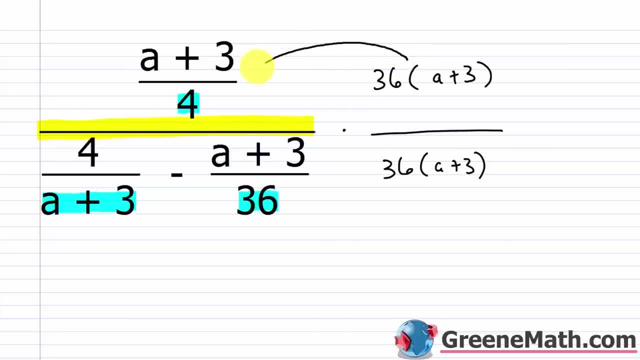 And so we're not changing the value. All right. So to kick this off, 36 times the quantity, a plus 3 multiplied by a plus 3 over 4, we can see that 36 would cancel with 4 and give us a 9.. 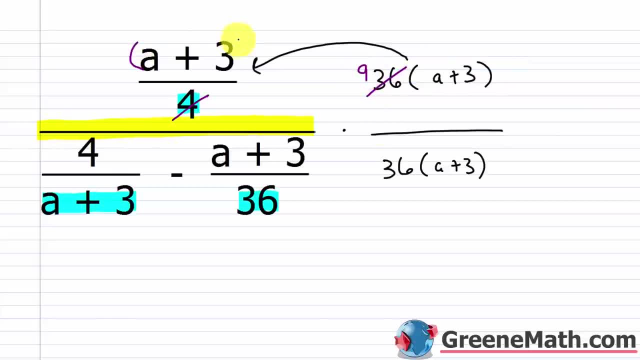 So essentially I have 9 times the quantity a plus 3, times the quantity a plus 3 again, which I can just simply write as 9 times the quantity a plus 3.. And this guy is squared Right. Or, if you want to write it out, you could do a plus 3, that quantity times a plus 3.. 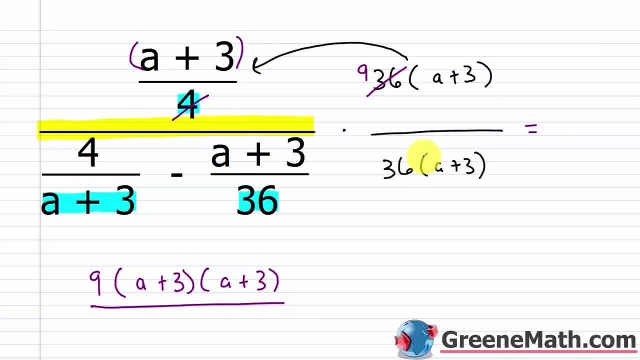 It does not matter. Okay, Then over. Now, this is going to distribute to each term, So it's going to start out right there And what's going to happen is, in that particular case, this a plus 3 is going to cancel with this a plus 3.. 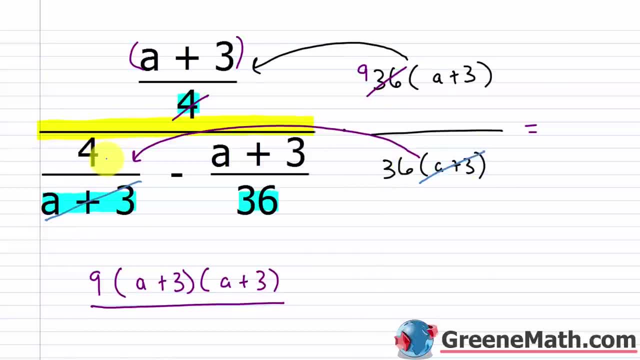 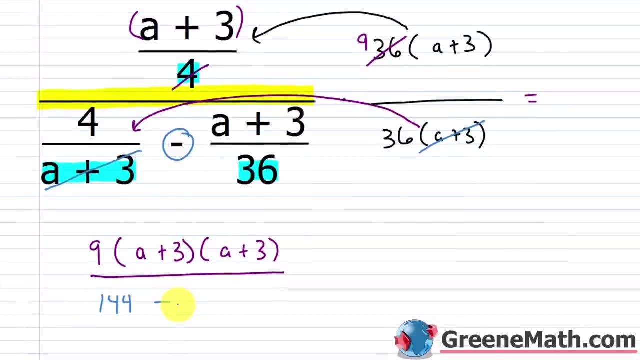 And then 36 times 4 is going to give me a 1.. Then I have a minus. So I have this minus sign. Now I'm going to use my distributive property for this term, And let me erase this part right here. 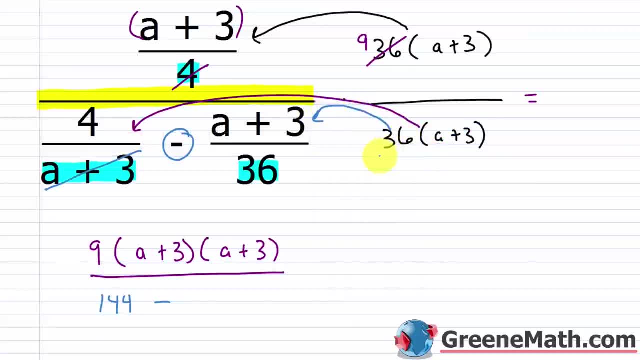 In this case the 36s are going to cancel And I'll have a plus 3 times a plus 3.. So those two quantities Again, I can write a plus 3, that quantity squared, Or I can write it out: a plus 3 times a plus 3.. 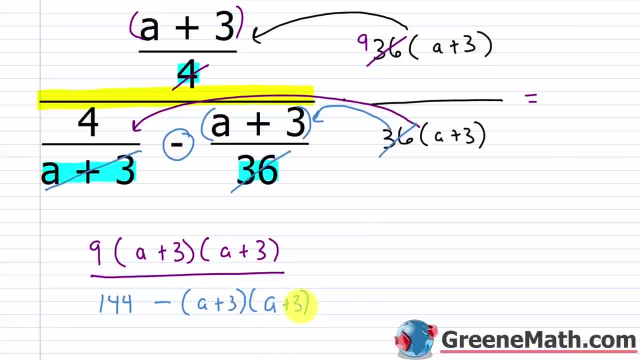 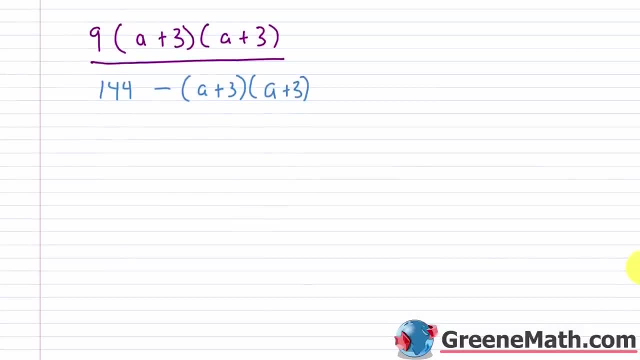 Okay. So now what we want to do is just simplify. So I'm going to write a plus 3 times a plus 3.. And what we want to do is just simplify. So we've gotten to that stage. now And again, I want to talk about a common mistake. 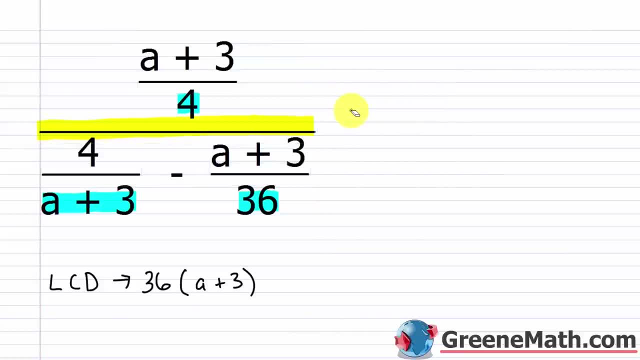 is at this point and i'm gonna put a multiplication symbol right here and i'm gonna be multiplying the numerator of the complex fraction by this thirty six times the quantity a plus three and i'm gonna do the same thing to the denominator and why is this legal before we move forward again this quantity over this quantity is equal to one right any non zero value over itself is one so thirty six times the quantity a plus three over thirty six times the quantity a plus three 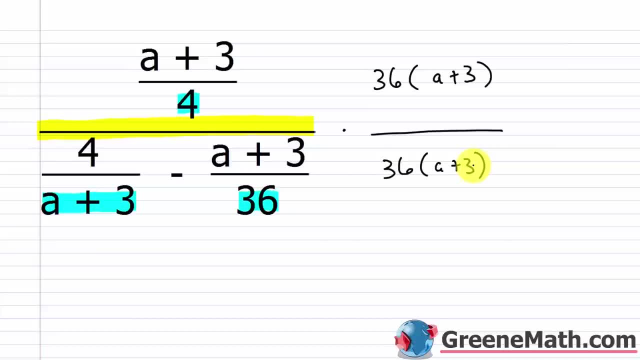 is one it's a complicated form of one but we are still multiplying by one and so we're not changing the value alright so to kick this off thirty six times the quantity a plus three multiplied by a plus three over four we can see that thirty six would cancel with four and give us a nine so essentially i have nine times the quantity a plus three times the quantity a plus three again which i can just simply write as nine times the quantity a plus three and this guy is squared 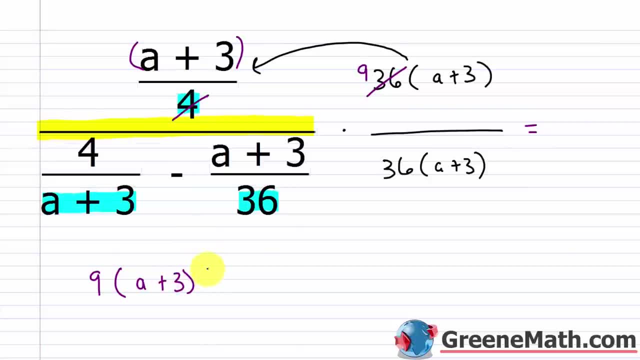 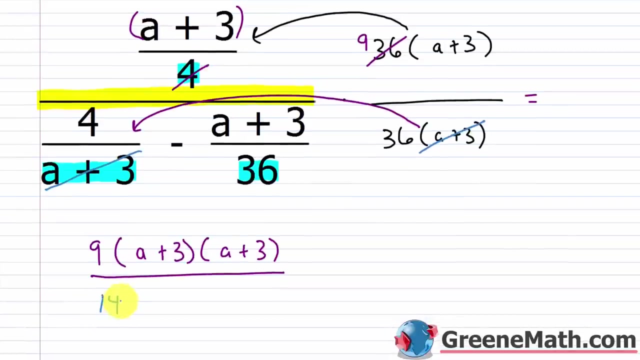 right or if you want to write it out you can do a plus three that quantity times a plus three does not matter okay then over now this is going to distribute to each term so it's gonna start out right there and what's gonna happen is in that particular case this a plus three is gonna cancel with this a plus three and then thirty six times four is gonna give me a hundred forty four then i have minus so i have this minus sign now i'm gonna use my 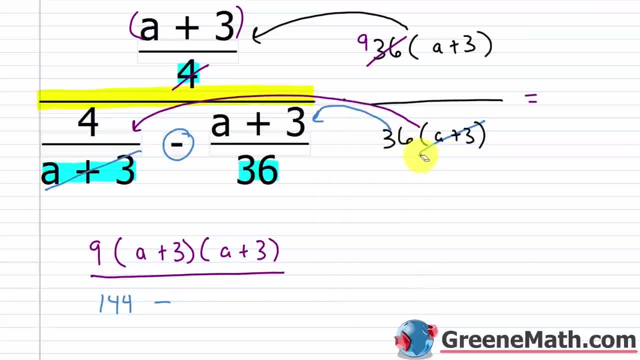 distributive property for this term and let me erase this part right here in this case the thirty sixes are gonna cancel and i'll have a plus three times a plus three so those two quantities again i can write a plus three that quantity squared or i can write it out a plus three times a plus three okay so now what we want to do is just simplify so we've gotten to that stage now 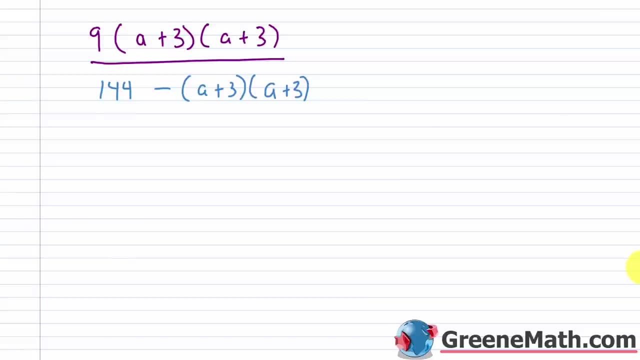 and again i want to talk about a common mistake i've talked about this in almost every video since i've kind of introduced 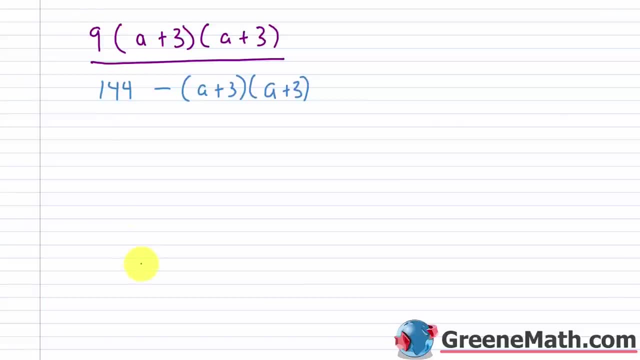 I've talked about this in almost every video since I've kind of introduced this, But I want you to understand. This is multiplication. here in the numerator, I'm multiplying 9 times the quantity a plus 3 times the quantity a plus 3.. 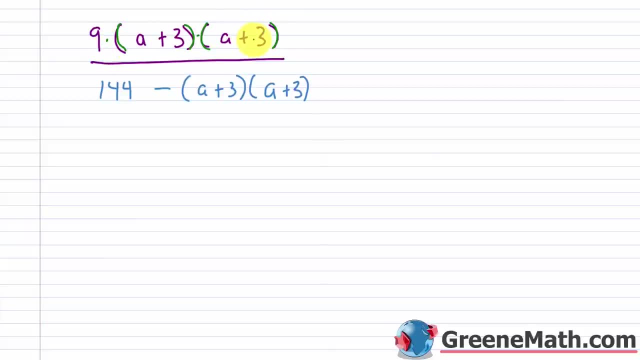 So I'm multiplying those three factors together. I don't have straight multiplication in the denominator Right. So what's going on here? I have 144, that is, subtracting away the product of a plus 3 times a plus 3.. So these are factors. 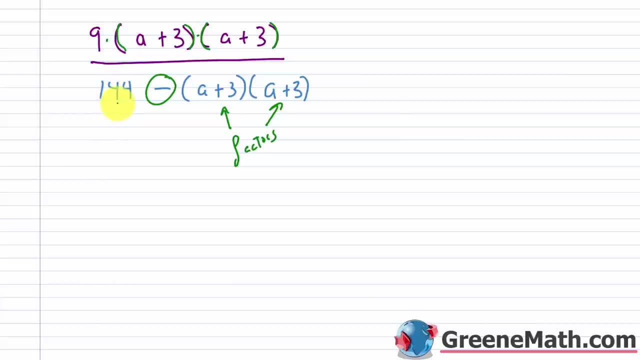 But this 144 is not a factor of anything Right. It's subtracting away the result of this multiplication. Again, if I don't have straight multiplication in both the numerator and the denominator, I can't go through and just cancel stuff. 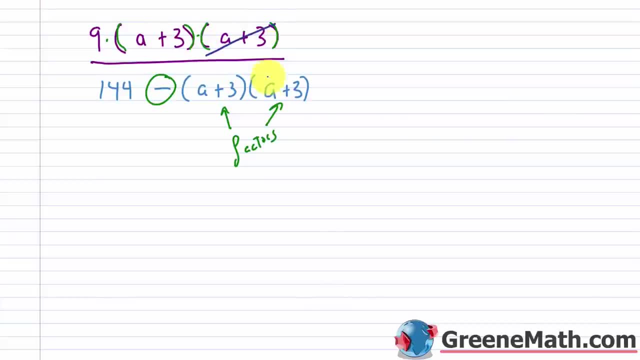 Right, I see students all the time. They'll say, okay, Cancel this with this and this with this, And then okay. Well, you know, 144 divided by 9 is 16.. So this with this and put a 16.. 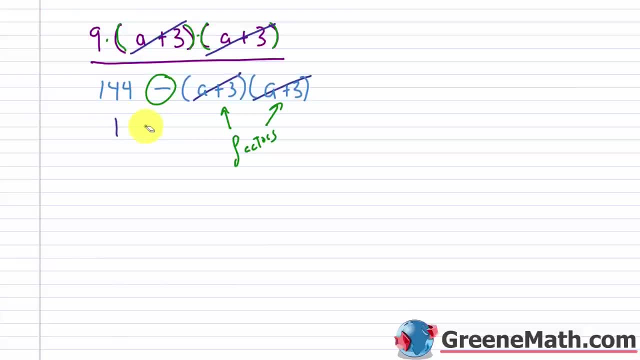 You cannot do that If you had- And let me just change this scenario up a little bit, Give you a different example- Something like 144 times the quantity a plus 3, times the quantity a plus 3.. Now these are all factors. 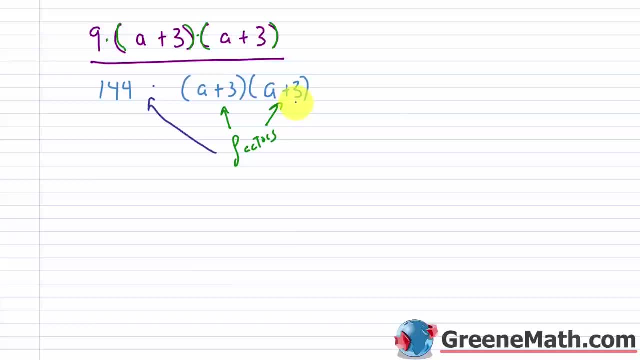 It's just straight multiplication here. So in this case I can go through and cancel this with this And this with this And this with this And get 16.. I'm going to end up with 1 16th there. 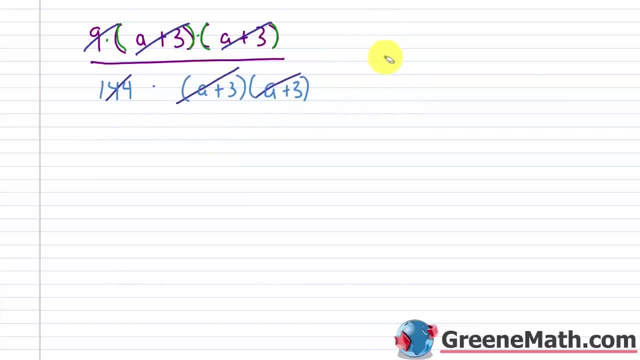 But that's not the situation we are presented with, And so again, we've got to act according to what we receive. So this is a minus sign here. 144 is subtracting away the result of the multiplication here, So please understand that you can't go through and just cancel that. 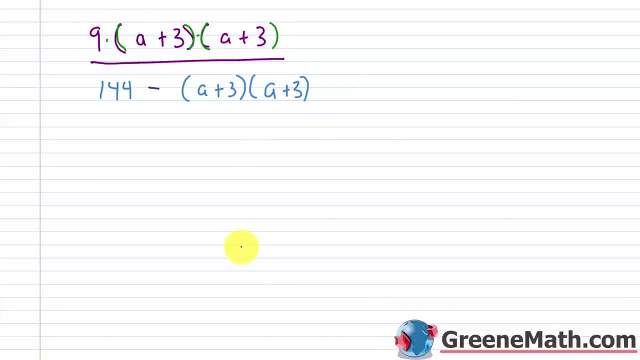 Okay. So now that we've kind of settled that, what could we do to simplify here? Well, in the numerator I'm just going to keep that in factored form. In the denominator I want to go through and use my special products formula to get the result for this. 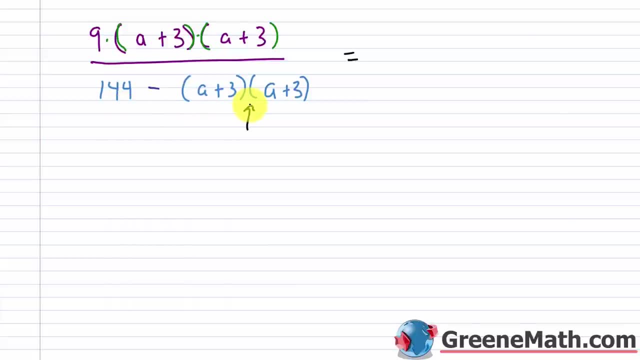 I'm going to subtract 144 minus that result And then I'm going to try to factor that guy and see if I can then cancel with something in the numerator. And I know this gets really, really tedious, But it's just something we have to do. 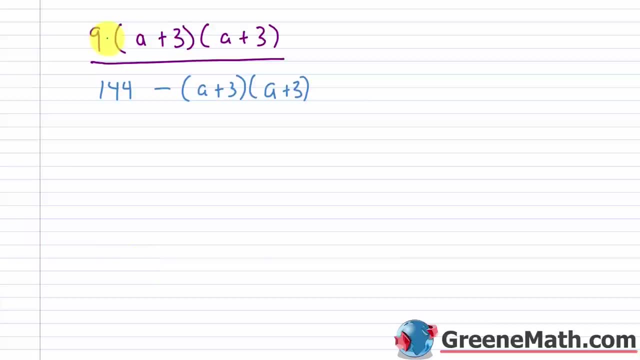 this but i want you to understand this is multiplication here in the numerator i'm multiplying nine times the quantity a plus three times the quantity a plus three so i'm multiplying those three factors together i don't have straight multiplication in the denominator i have a subtraction sign here i have a hundred forty four that is subtracting away the product of a plus three times a plus three but this a hundred forty four 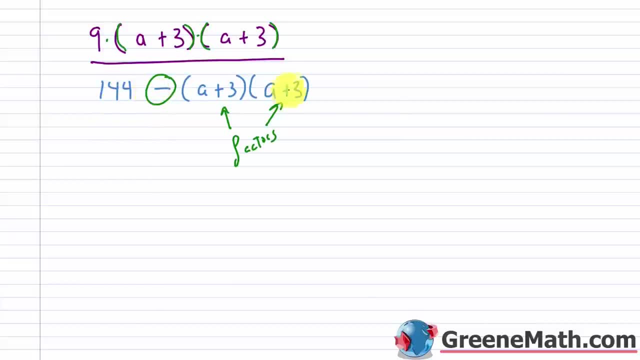 is not a factor of anything it's subtracting away the result of this multiplication again if i don't have straight multiplication in both the numerator and the denominator i can't go through and just cancel stuff right i see students all the time they'll say okay well i can cancel this with this and this with this and then okay well you know a hundred forty four divided by nine is sixteen so this with this and put a sixteen you cannot do that if you had and let me just change this scenario up a little bit give you a different 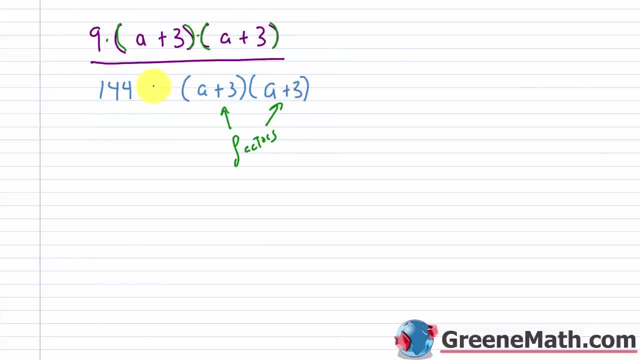 example something like a hundred forty four times the quantity a plus three times the quantity a plus three now these are all factors it's just straight multiplication here so in this case i can go through and cancel this with this and this with this and this with this and get sixteen i'm going to end up with one sixteenth there but that's not the situation we are presented with 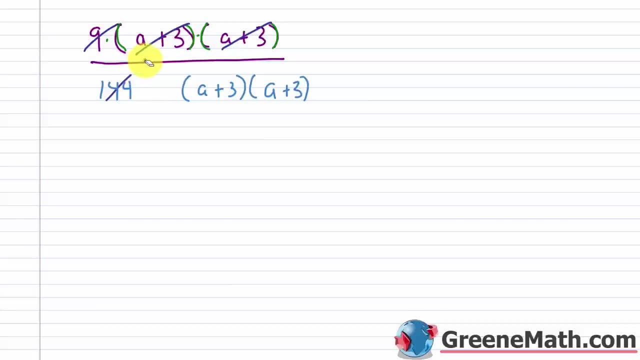 and so again we've got to act according to what we receive so this is a minus sign here a hundred forty four is subtracting away 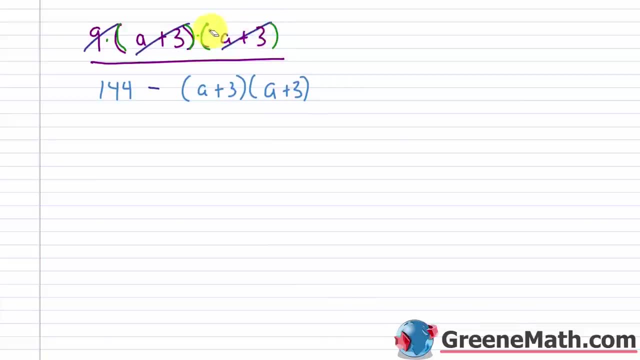 the result of the multiplication so please understand that you can't go 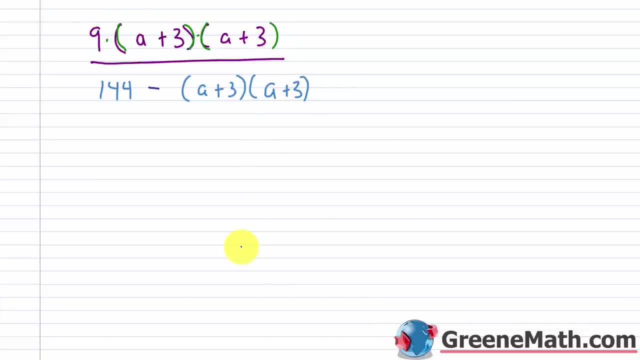 through and just cancel there okay so now that we've kind of settled that 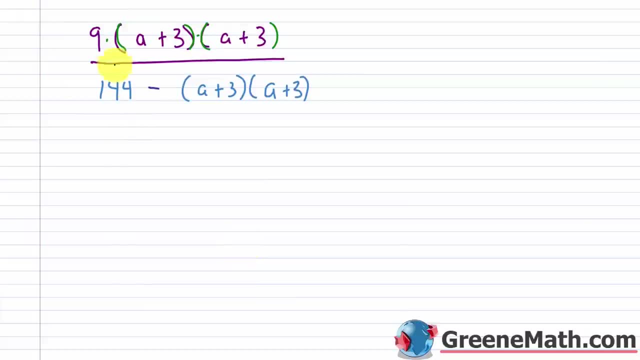 what could we do to simplify here well in the numerator i'm just going to keep that in factored form in the denominator 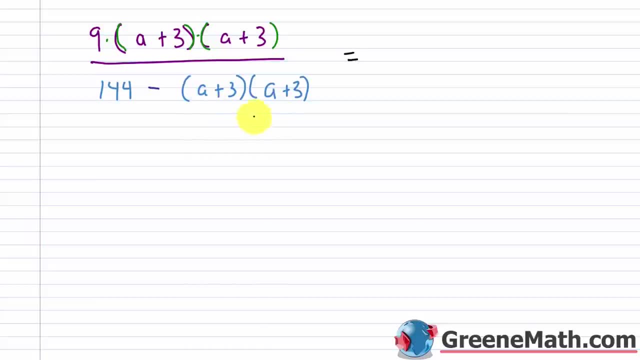 i want to go through and use my special products formula to get the result for this i'm going to subtract a hundred forty four minus that result and then i'm going to try to factor that guy and see if i can then cancel with something in the numerator 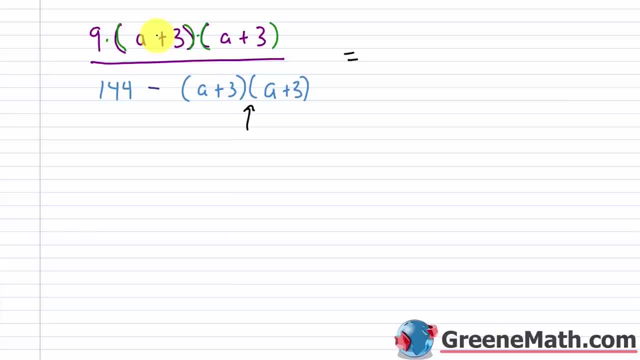 and i know this gets really really tedious but it's just something we have to do alright so i'm just going to copy the numerator nine times the quantity a plus three times the quantity a plus three and then over so the formula for this a times a is a squared then the middle term i know that i'd have two times a times three so that's plus six a and then the final would be three squared or nine now here's the kicker 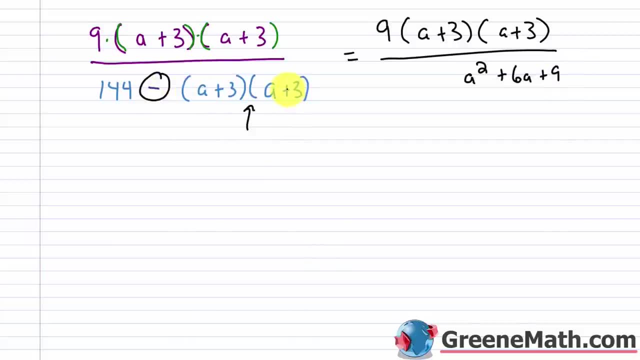 i am subtracting away the result of this okay so that means i'm subtracting each and every term away or i'm subtracting the whole thing away so one good way is to put this inside of parentheses and then when you drop the parentheses you're going to change the sign of each term so i'd have negative a squared minus six a minus nine and don't forget that you have the hundred forty four out in front and then what i'm going to do here is i'm going to subtract a hundred forty four minus nine that's going to give me positive a hundred thirty five so i'm going to write this 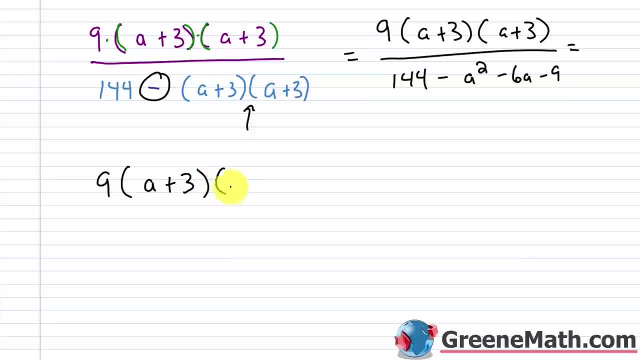 as nine times the quantity a plus three times the quantity a plus three again and then over we have negative a squared then minus six a and again a hundred forty four minus nine is plus 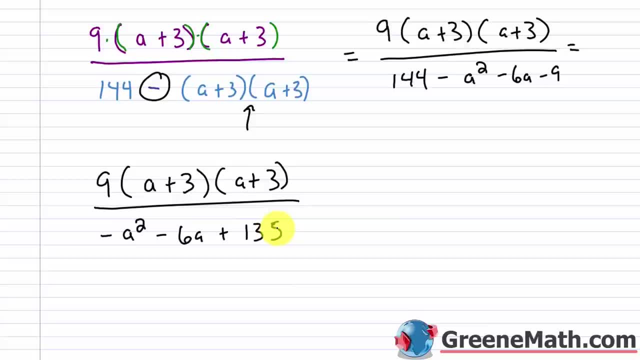 one hundred thirty five now the question would be can i factor this and then cancel 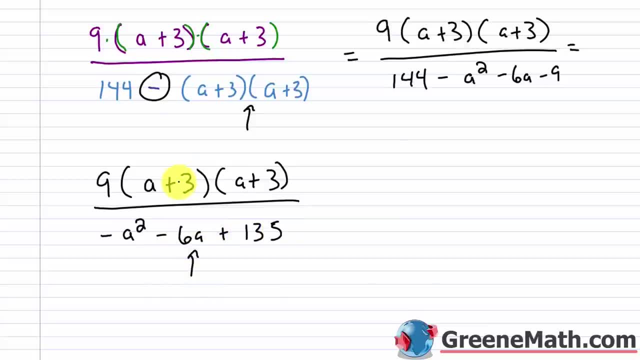 one of those factors with something up here well i'm going to tell you that you can factor it but nothing's going to cancel we're going to go through and factor it anyway so the 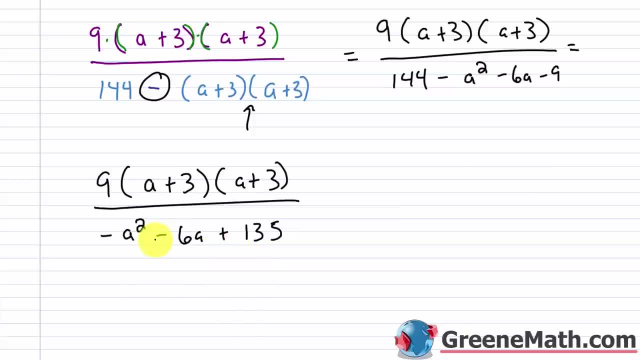 first thing i'm going to do to make this easy for you i'm going to factor out a negative one so the way that i do that is i just put a negative one out in front of parentheses and i change the sign of each term inside so this was negative now it's positive this was negative now it's going to be positive and this was positive now it's going to be negative so now it's very easy for me to factor this because i have a leading coefficient on a squared that's positive one and that's what we're used to 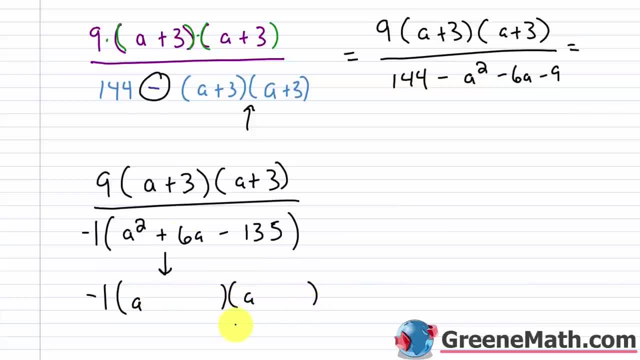 and so give me two integers whose sum is positive 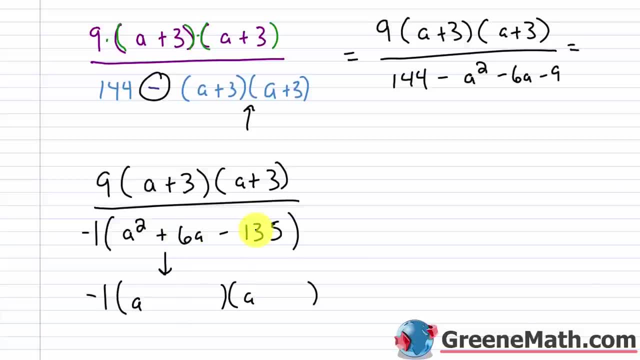 six and whose product is negative one hundred thirty five 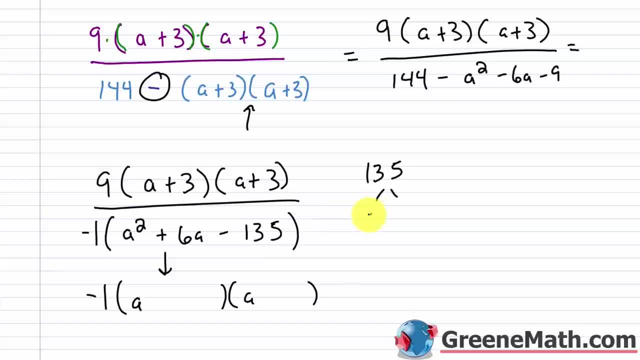 so if i think about a hundred thirty five pretty easy it's what twenty seven 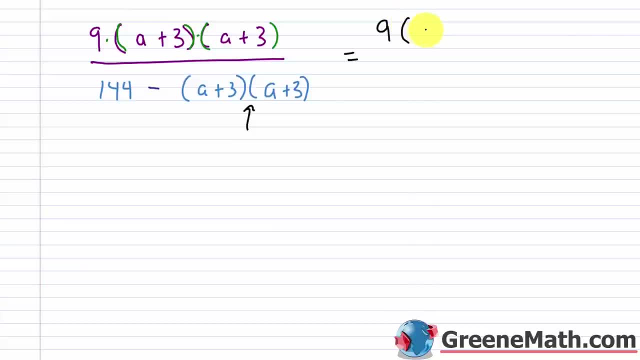 All right, So I'm just going to copy the numerator: 9 times the quantity a plus 3, times the quantity a plus 3.. And then over. So the formula for this a times a is a squared, Then the middle term. I know that I'd have 2 times a times 3.. 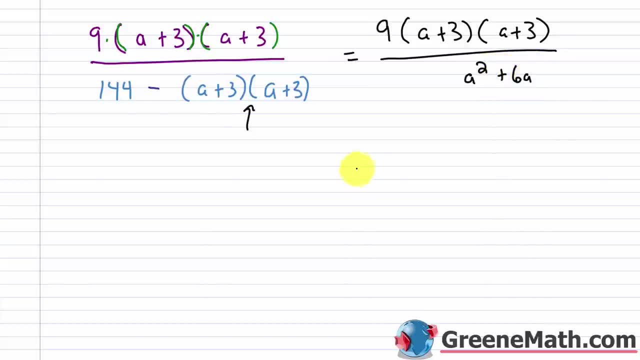 So that's plus 6a, And then the final would be 3 squared or 9.. Now here's the kicker: I am subtracting away the result of this. Okay, So that means I'm subtracting each and every term away, or I'm subtracting the whole thing away. 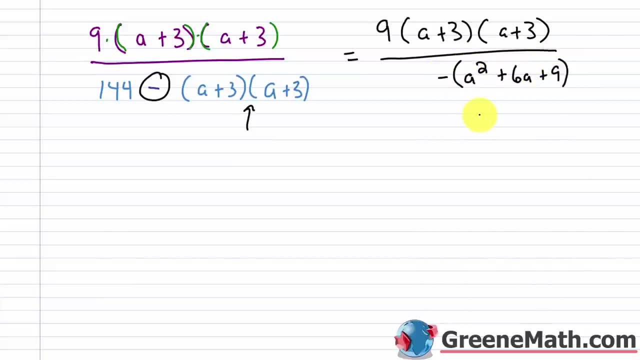 So one good way is to put this inside of parentheses And then when you drop the parentheses, you're going to change the sign of each term. So I'd have negative a squared minus 6a minus 9.. And don't forget that you have the 144 out in front. 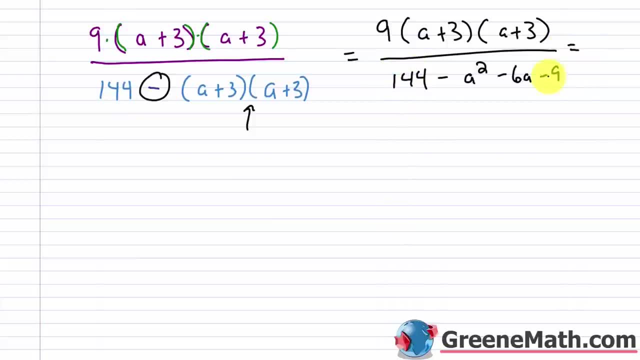 And then what I'm going to do here is I'm going to subtract 144 minus 9.. That's going to give me positive 135.. So I'm going to write this as 9 times the quantity a plus 3 times the quantity a plus 3 again. 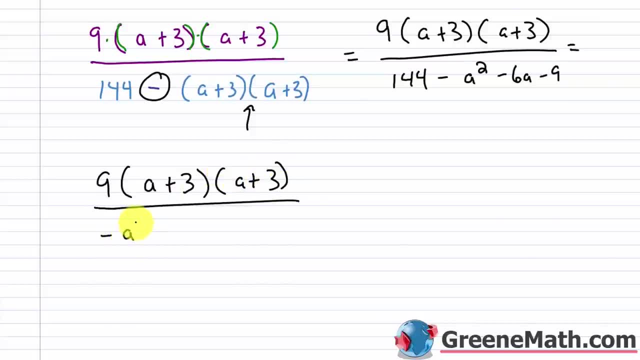 And then over We have negative a squared, Then minus 6a, And again 144 minus 9 is plus 135.. Now the question would be: can I factor this and then cancel one of those factors with something up here? 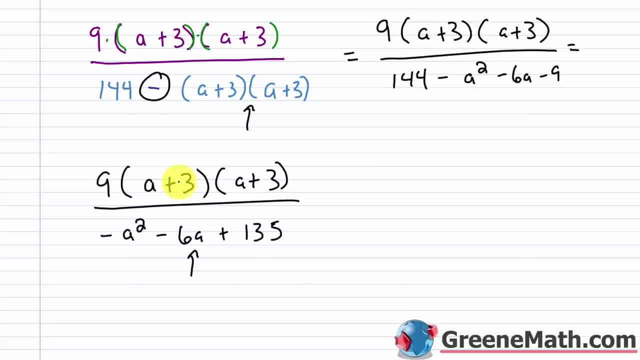 Well, I'm going to tell you that you can factor it, but nothing's going to cancel. We're going to go through and factor it anyway. So the first thing I'm going to do, to make this easy for you, I'm going to factor out a negative 1.. 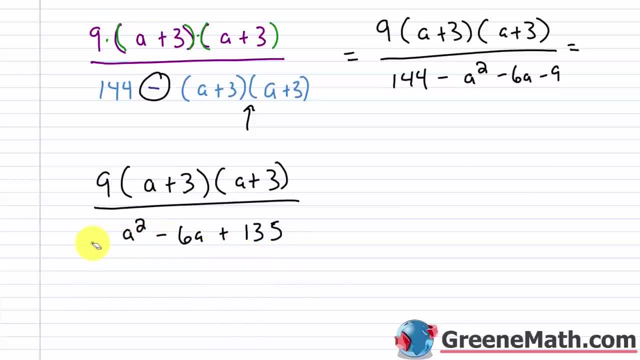 So the way that I do that is I just put a negative 1 out in front of parentheses And I change the sign of each term inside. So this was negative, Now it's positive. This was negative, Now it's going to be positive. 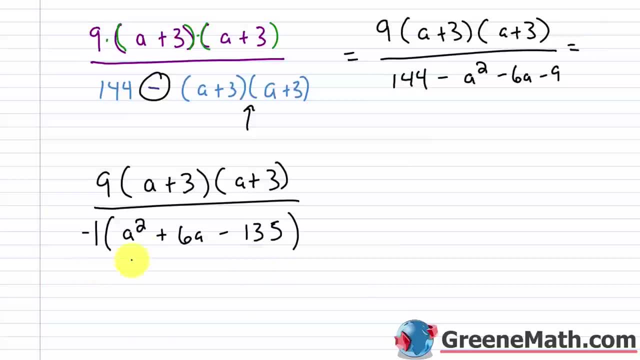 And this was positive. Now it's going to be negative. So now it's very easy for me to factor this, because I have a leading coefficient on a squared that's positive: 1. And that's what we're used to. And so give me two integers whose sum is positive, 6, and whose product is negative, 135.. 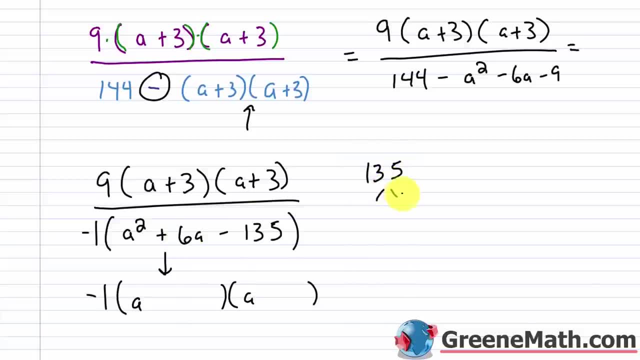 So if I think about 135.. Pretty easy, It's what? 27 times 5.. 27 is 9 times 3.. 9 is 3 times 3.. And so if I think about possible factors, the one that jumps out right away is what? 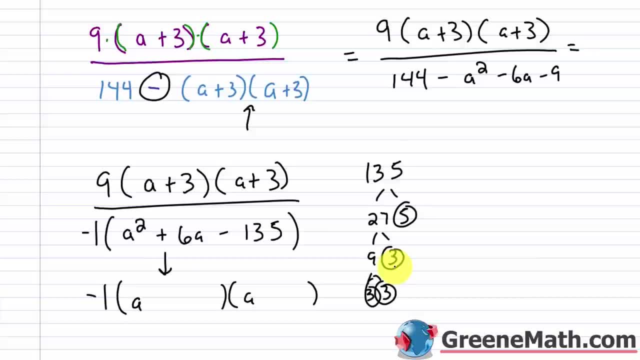 15 and 9.. Right 15 and 9.. So if I did positive 15 and negative 9.. So plus 15 and negative 9. The sum is going to be positive 6. The product's going to be negative 135.. 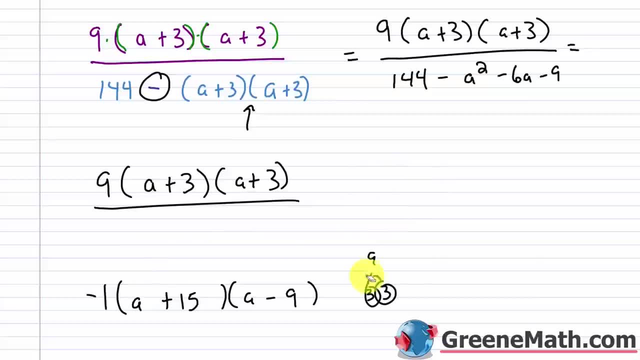 So let's just erase this and this And we'll just kind of drag this up here And what you're going to see is that nothing is actually going to cancel here. I don't have any common factors. A plus 3, that quantity. 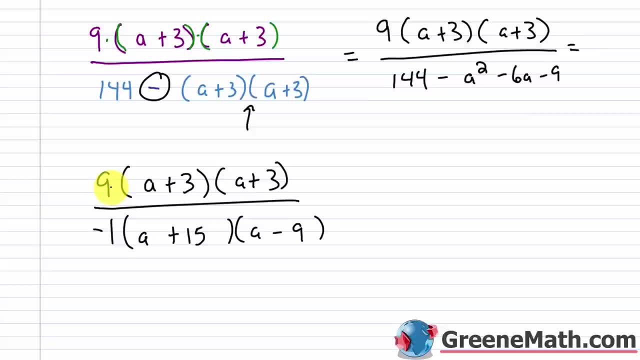 A plus 3, that quantity And 9 are my factors in the numerator Negative, 1. A plus 15. And A minus 9 are my factors in the denominator. There's nothing I can cancel, So for most teachers you would just report your answer in this format. 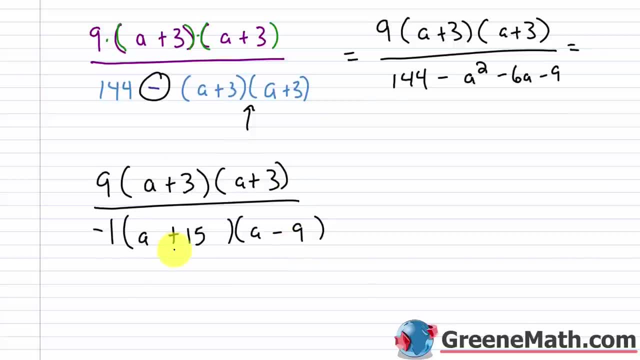 For others. they want you to go through and kind of multiply through And kind of multiply everything together So we can do that real quick. So 9 is going to be multiplied by the result of this. So we know that this is A squared plus 6A plus 9.. 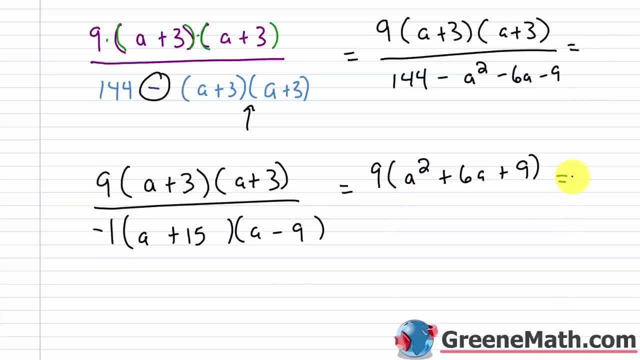 Then if I do the multiplication- Let me kind of just do this down here- That would be 9A squared plus 54A plus 81.. So that's going to be my numerator. Then this is over Down here. we just factored this. 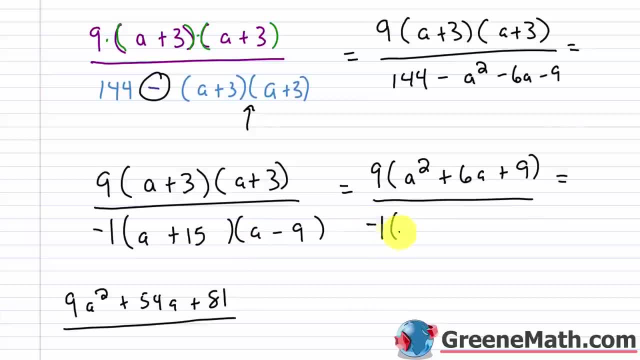 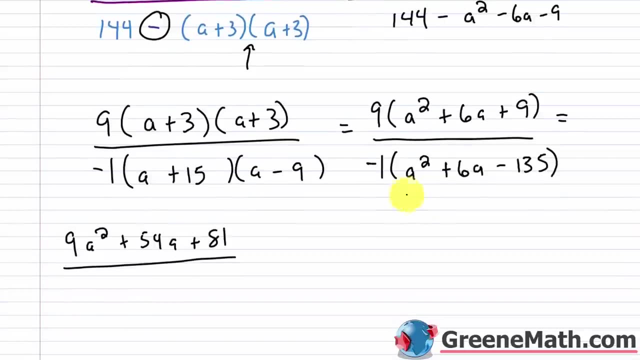 So we know what it is. It's negative 1 times. Again, this would be A squared plus 6A And then minus 135.. And then a few things you can do. You can write the denominator as A squared plus 6A, minus 135.. 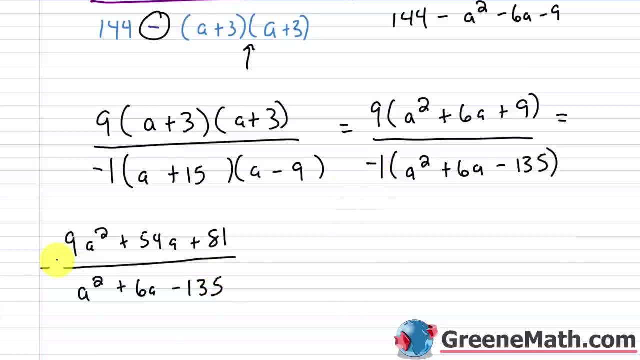 And just put this negative out in front. You'll see that in a lot of answers. Or you can just make each term the opposite of what it is. So you could say: this is negative A squared And then minus 6A And then plus 135.. 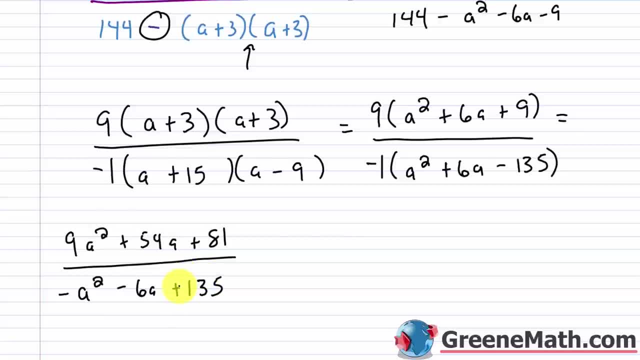 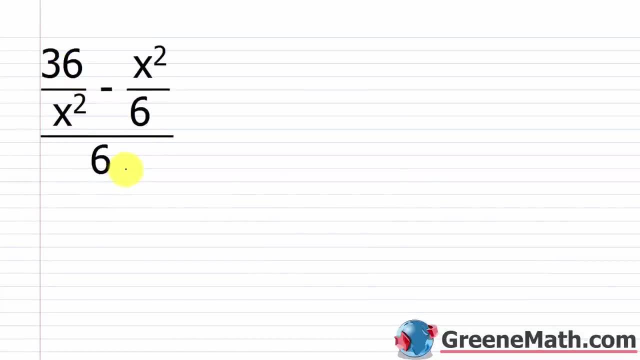 There's quite a few different ways you could write this. It's just a matter of what your teacher wants from you. Alright, let's take a look at another one. We have 36 over X squared minus X squared over 6.. And then this is over 6.. 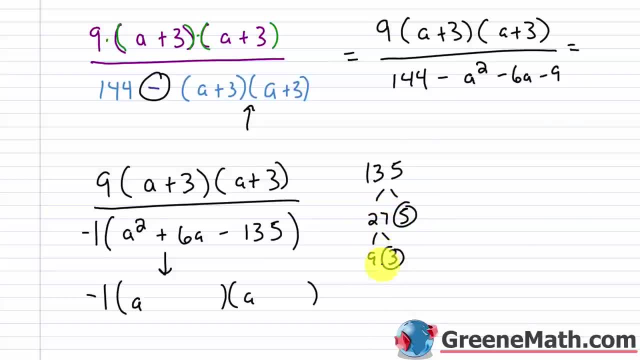 times five twenty seven is nine times three nine 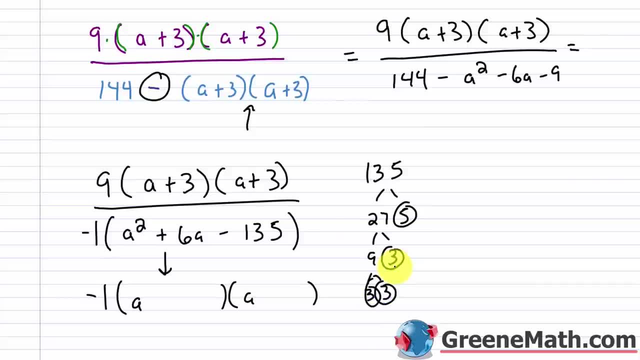 is three times three and so if i think about possible factors 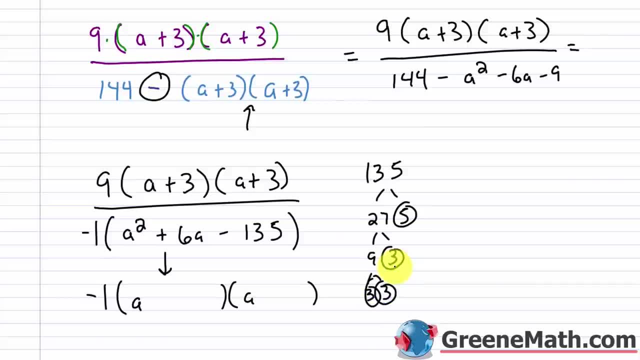 the one that jumps out right away is what fifteen and nine right fifteen and nine so if i did positive 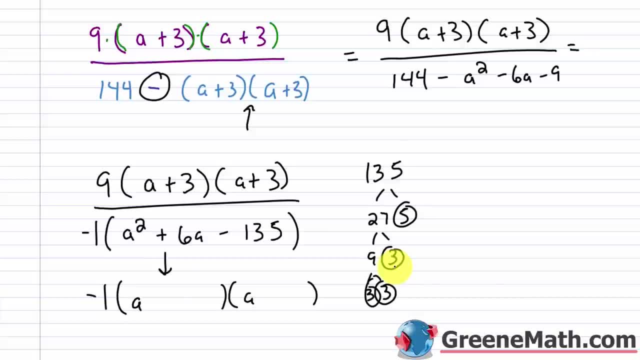 fifteen and negative nine so plus fifteen 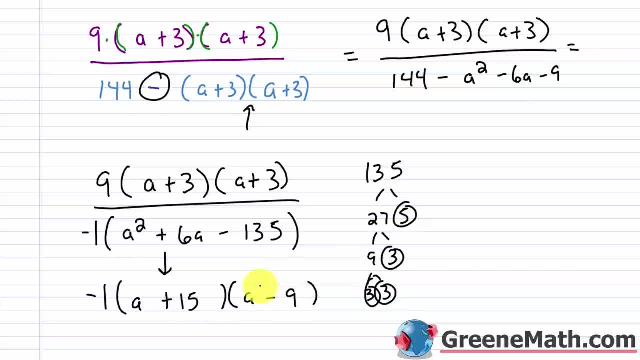 and negative nine the sum is going to be positive six the product is going to be negative one hundred thirty five so 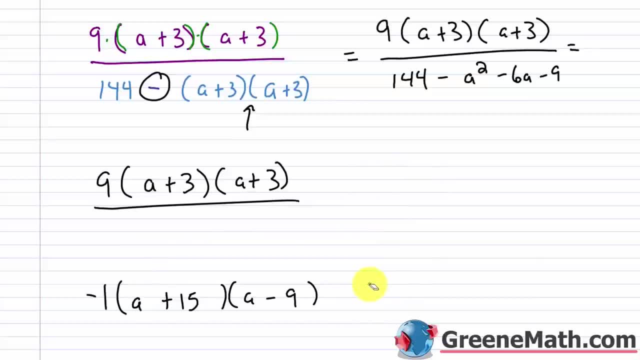 let's just erase this and this we'll just kind of drag 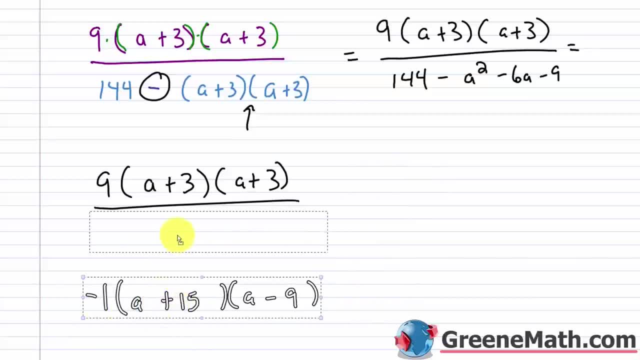 this up here and what you're going to see is that nothing is actually going 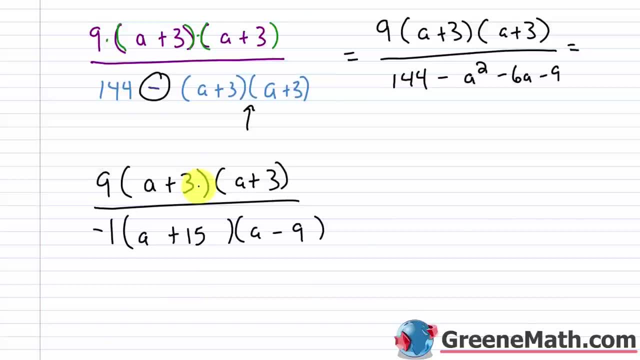 to cancel here i don't have any common factors a plus three that quantity a plus three that quantity and nine are my factors in the numerator negative one a plus fifteen and a minus nine are my factors in the denominator there's nothing i can cancel so 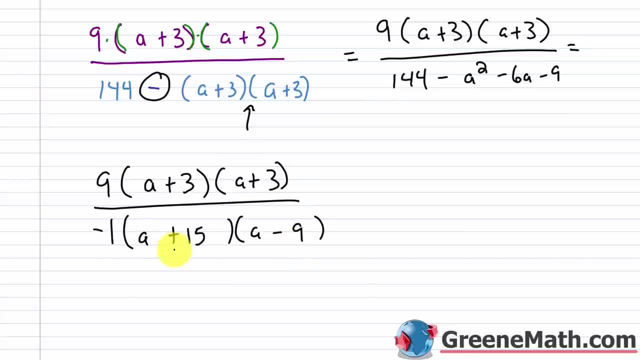 for most teachers you would just report your answer in this format for others they want you to go through and kind of multiply everything together so we can do that real quick so nine is going to be multiplied by the result of this so we know that this is a squared plus six a plus nine then if i do the multiplication let me kind of just do this down here that would be nine a squared plus fifty four a plus eighty one so that's going to be my numerator 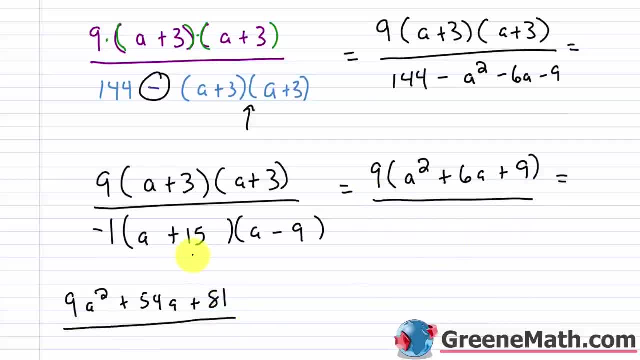 then this is over down here we just factored this so we know what it is it's negative one times 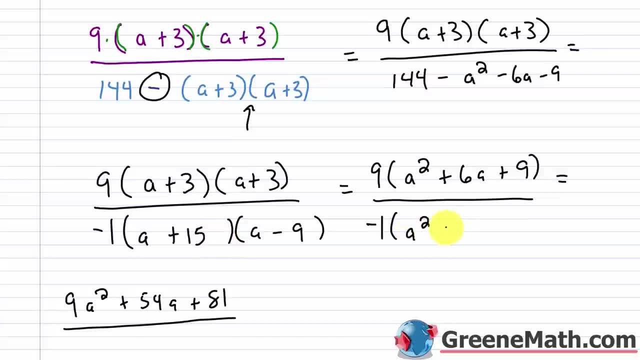 again this would be a squared plus six a and then minus one hundred thirty five and then a few things 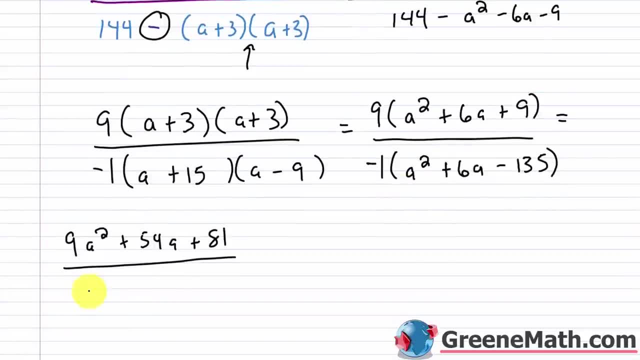 you can do you can write the denominator as a squared plus six a minus one hundred thirty five and just put this negative out in front you'll see that in a lot of answers 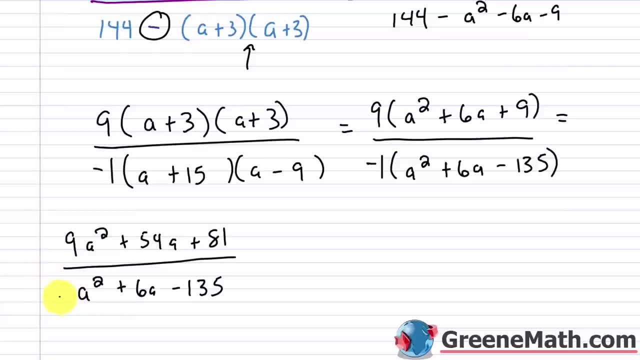 or you can just make each term the opposite of what it was so you can say okay this is negative a squared and then minus six a and then plus one hundred thirty five there's quite a few different ways you could write this it's just a matter of what your teacher wants from you alright let's take a 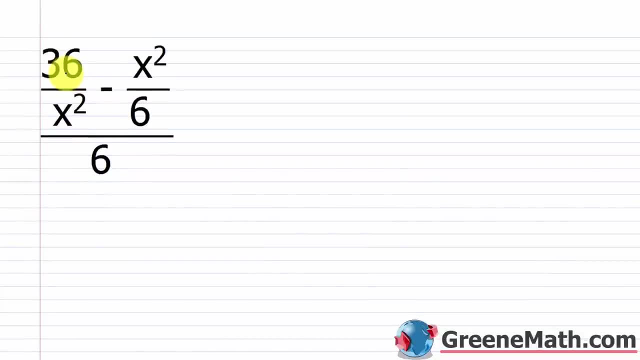 look at another one we have thirty six over x squared minus x squared over six and then this is over six now don't get confused with this one 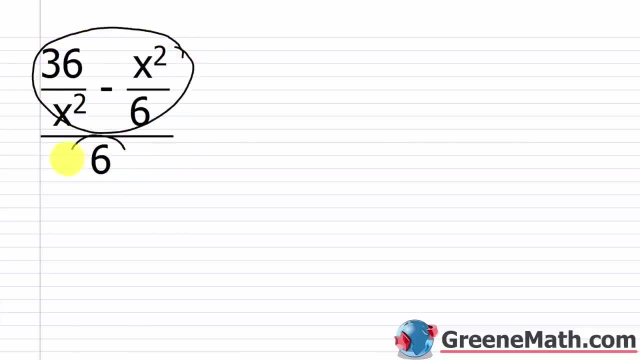 this is your numerator for the complex fraction this is your denominator okay the denominator does not have to have a fraction involved it can just be a number six 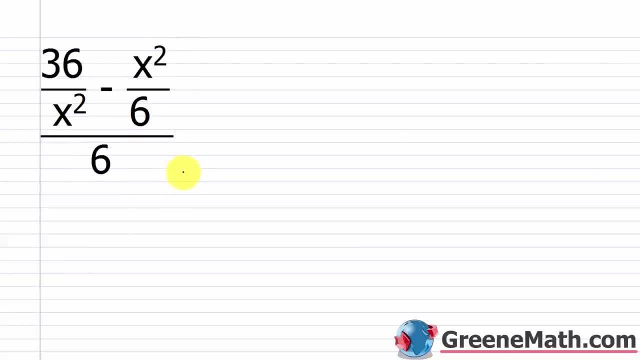 but in order to not confuse yourself here go ahead and write it as six over one so now it's clear what i'm thinking about six over one the denominator is a one and then for thirty six over x squared the denominator is x squared and then for this guy x squared over six the denominator is a six so what would the lcd be it would just be six x squared so then i can erase all this and just say okay i'm going to multiply this by six x squared over six x squared so 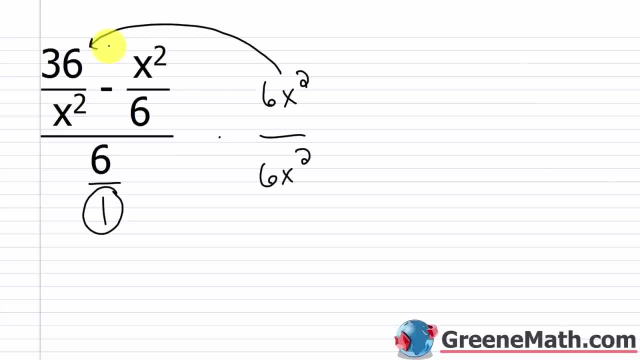 if i do this six x squared times thirty six over x squared the x squares would cancel this would cancel with this and i'd have six times thirty six which is two hundred sixteen 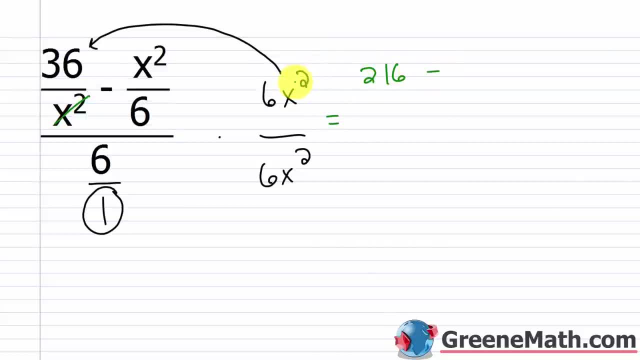 then minus you kind of erase this real quick you'd have six x squared times x squared over six the sixes would cancel you'd have x to the fourth power so x to the fourth power and this is over if i have six times six x squared that's just thirty six x squared so 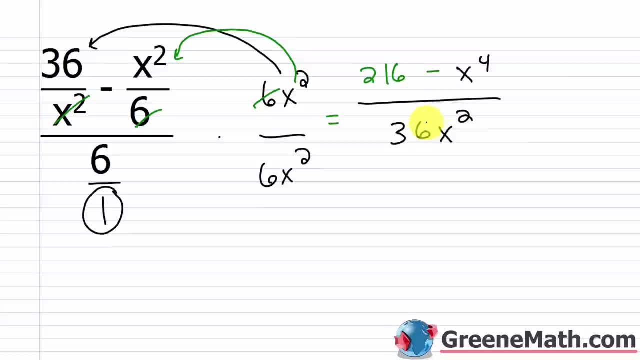 is there anything that i can do to factor this guy well if two hundred sixteen was a perfect square i could use the difference of two squares there but it's not so there's not really anything i can do 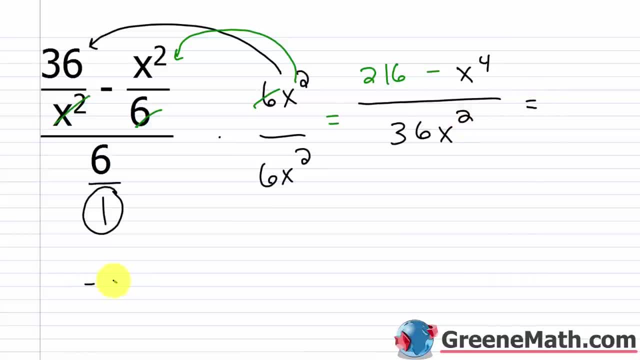 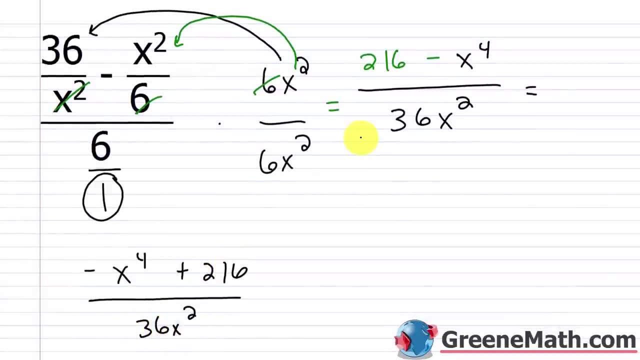 a lot of you will like to flip your answer around and say okay well this is negative x to the fourth power plus two hundred sixteen over thirty six x squared that's fine either way is acceptable alright let's take a look 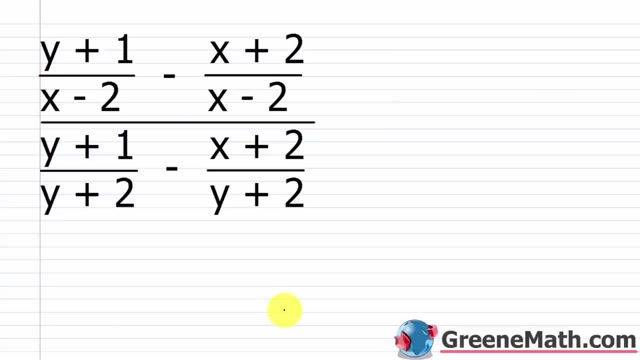 at one final problem i think that all of us can agree that this is a much faster method 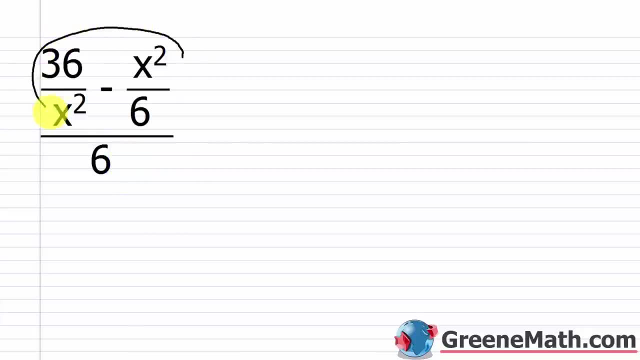 Now, don't get confused with this one. This is your numerator for the complex fraction. This is your denominator. The denominator does not have to have a fraction involved, It can just be a number 6.. But in order to not confuse yourself here, 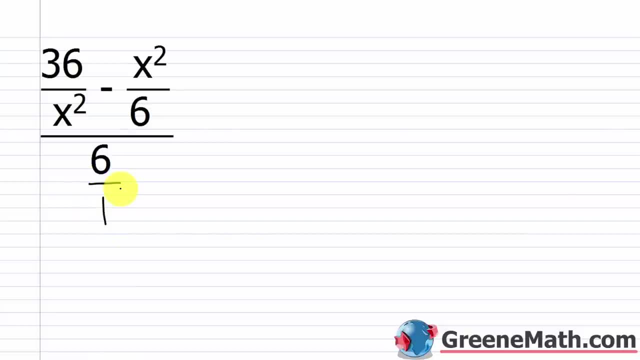 Go ahead and write it as 6 over 1.. So now it's clear when I'm thinking about 6 over 1.. The denominator is a 1.. And then, for 36 over X squared, The denominator is X squared, And then for this guy, X squared over 6.. 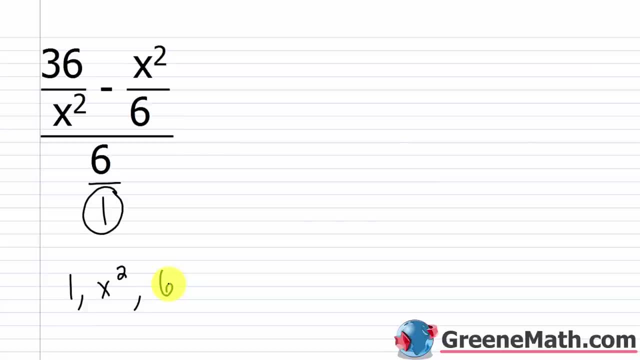 The denominator is a 6. So what would the LCD be? It would just be 6X squared. So then I can erase all this And just say: okay, I'm going to multiply this by 6X squared Over 6X squared. 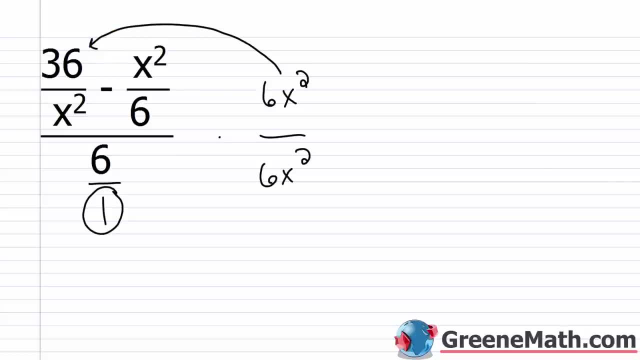 So if I do this, 6X squared times 36 over X squared, The X squareds would cancel. This would cancel with this And I'd have 6 times 36.. Which is 216.. Then minus And kind of erase this real quick. 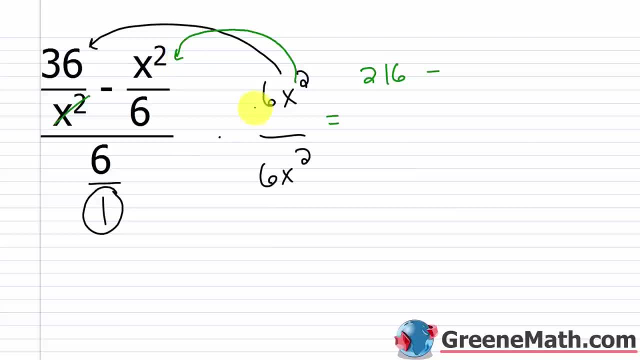 You'd have 6X squared times X squared over 6.. The 6's would cancel. You'd have X to the 4th power, So X to the 4th power And this is over If I have 6 times 6X squared. 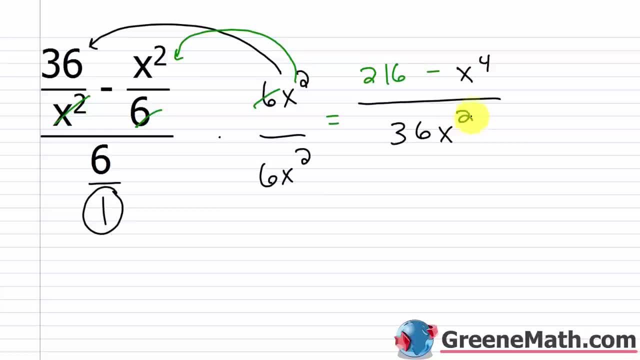 That's just 36X squared. So Is there anything that I can do To factor this guy? Well, if 216 was a perfect square, I could use the difference of two squares there, But it's not, So there's not really anything I can do. 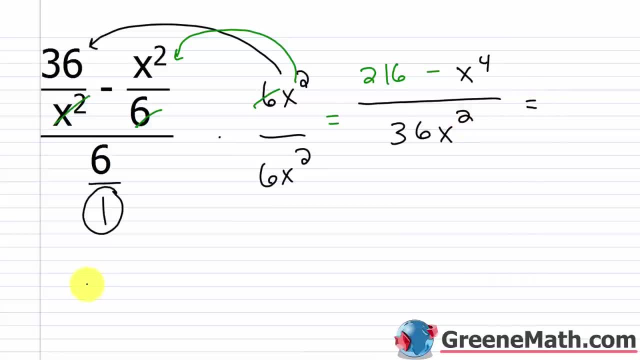 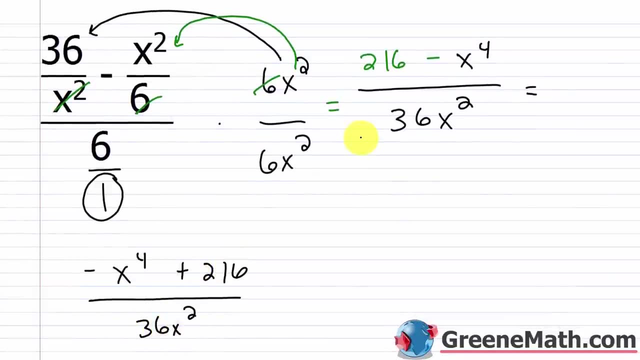 A lot of you will like to flip your answer around And say: okay, Well, this is negative. X to the 4th power Plus 216.. Over 36X squared, That's fine. Either way is acceptable. I think that all of us can agree that. 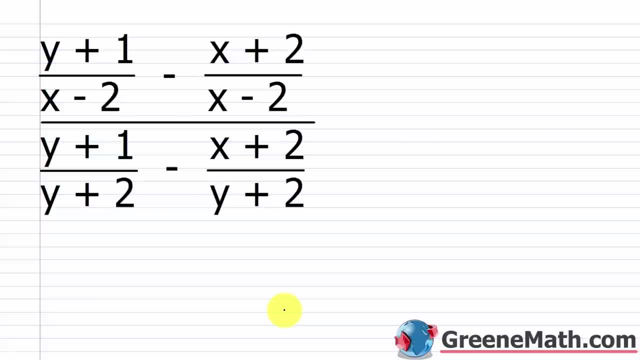 This is a much faster method. You just have to be able to understand it. Again, it doesn't take long to understand it. You just have to be able to identify What denominators you're looking at To produce your LCD. So for this one, we have 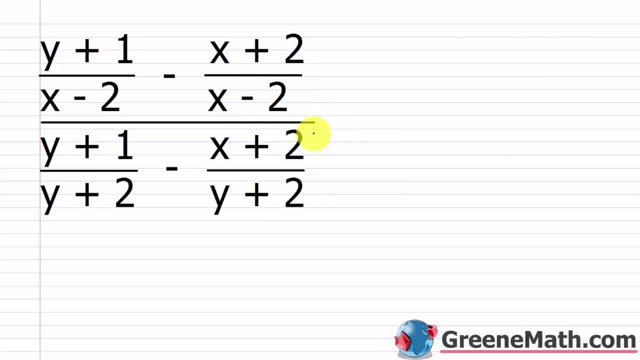 Y plus 1 over X minus 2.. Minus X plus 2 over X minus 2.. And then this is over Y plus 1 over Y plus 2.. Minus X plus 2 over Y plus 2.. So what I'm looking at here 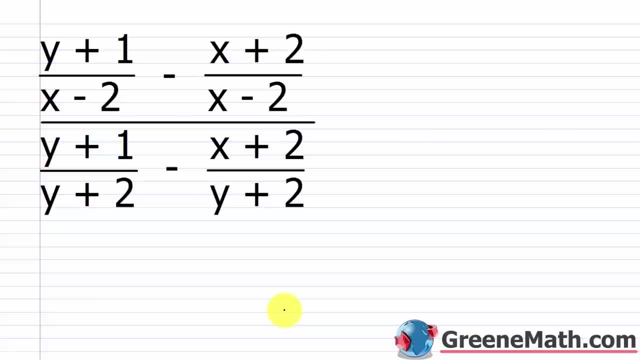 you just have to be able to understand it again it doesn't take long to understand you just have to be able to identify what denominators you're looking at to produce your lcd so for this one we have y plus one over x minus two 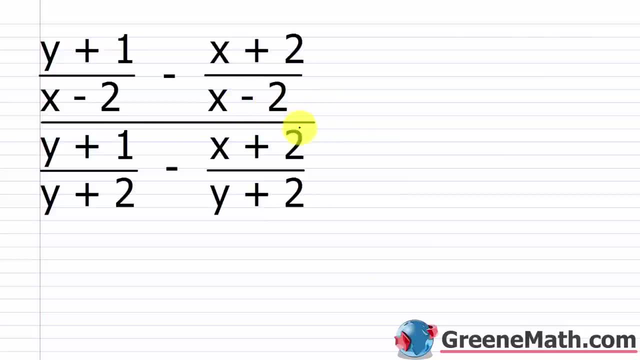 minus x plus two over x minus two and then this is over y plus one over y plus two minus x plus two over y plus two so what i'm looking at here is an lcd 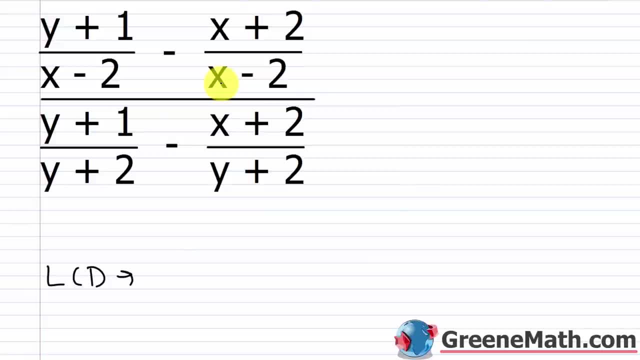 that's what the denominators here are the same x minus two in each case 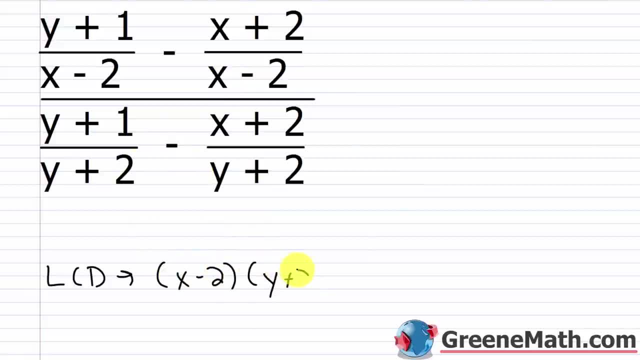 the denominators here are the same y plus two in each case so all i can do is just multiply the denominators together i can't do any better than that but again notice how in the numerator of the complex fraction i'm looking at this denominator this denominator in the denominator of the complex fraction i'm looking at this denominator and this denominator so again you're looking at all the denominators involved of that complex fraction so this one this one this one and this one alright so once we have our lcd 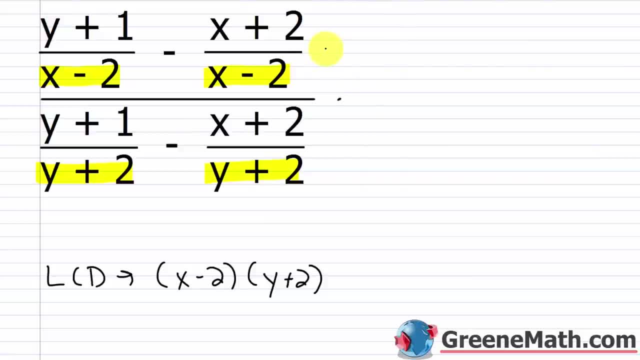 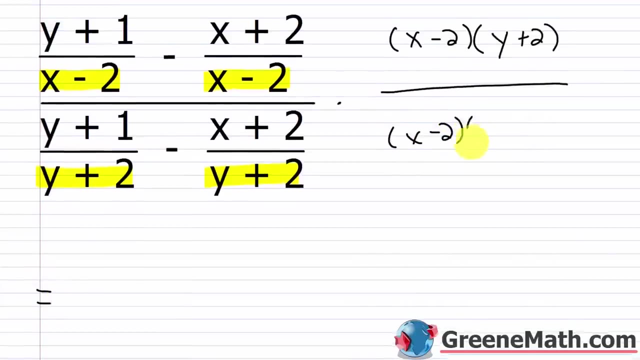 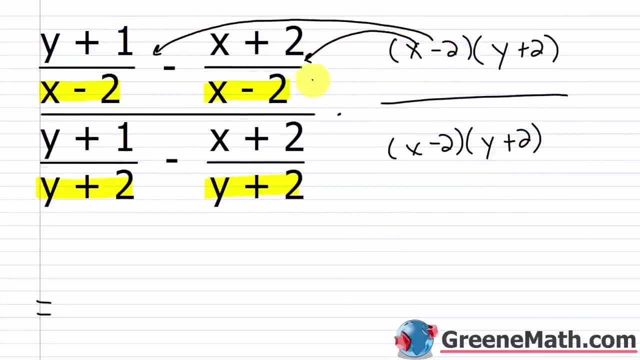 going all we need to do is multiply the numerator and denominator of the complex fraction by that lcd so x minus two that quantity times y plus two now this is pretty simple to do because in this case when i multiply here in each case the x minus two is going to cancel and i'm just going to be left with the y plus two times the numerator in other words this is going to cancel with that in each case so 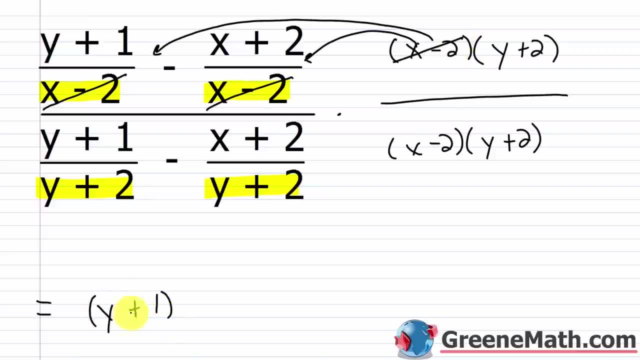 y plus two times y plus one let's write that out and i'm going to leave it in factored form for now and then i'm subtracting away and you can put that inside of brackets or just remember that you're subtracting the whole thing away you have y plus two times x plus two right those two quantities 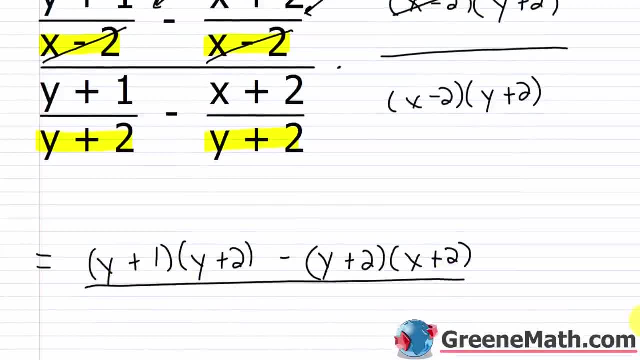 alright then this is over for the next one in a similar way the 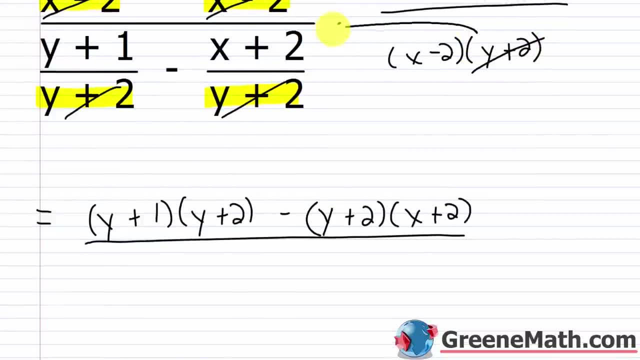 y plus two is going to cancel here and here right when i do the multiplication 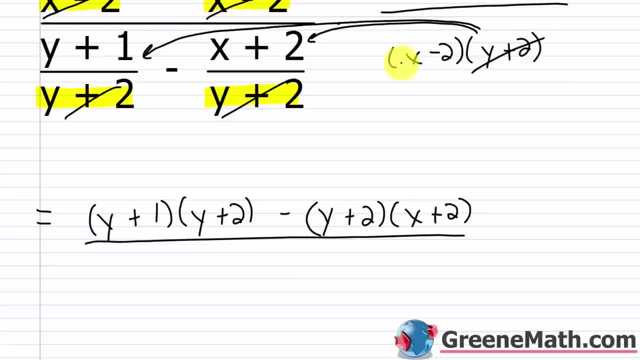 to each so i'm going to be left with x minus two times y plus one 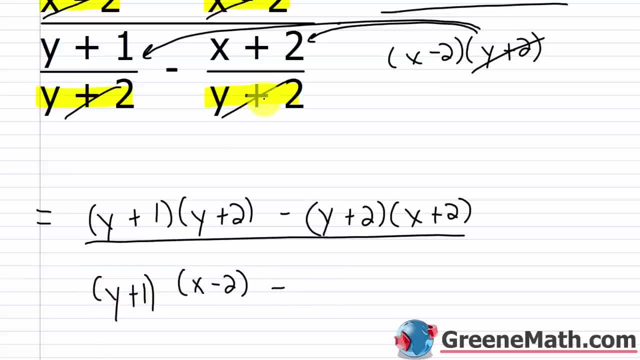 and then minus in this case i'll have x plus two and then times x minus two 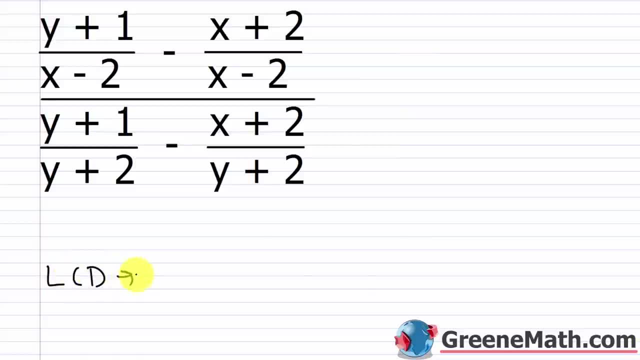 Is an LCD. That's what. The denominators here are the same: X minus 2 in each case. The denominators here are the same: Y plus 2 in each case. So all I can do Is just multiply the denominators together. 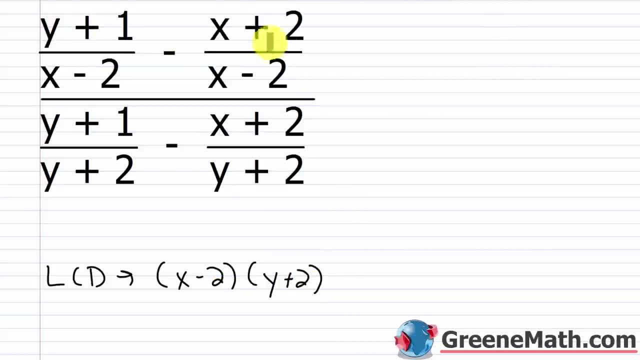 I can't do any better than that, But again, notice how, In the numerator of the complex fraction, I'm looking at this denominator, This denominator. In the denominator of the complex fraction, I'm looking at this denominator And this denominator. 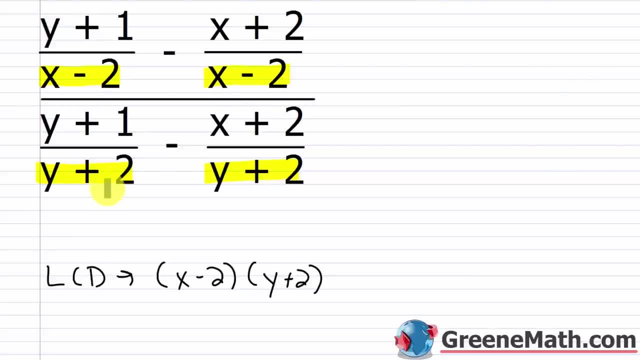 Of that complex fraction. So this one, this one, this one and this one. Alright, So once we have our LCD going, All we need to do is multiply The numerator and denominator of the complex fraction By that LCD. So X minus 2 at quantity. 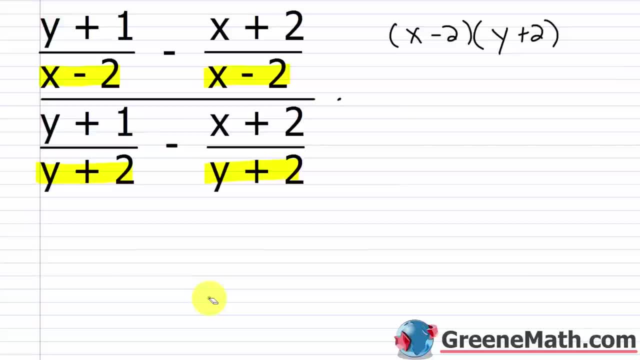 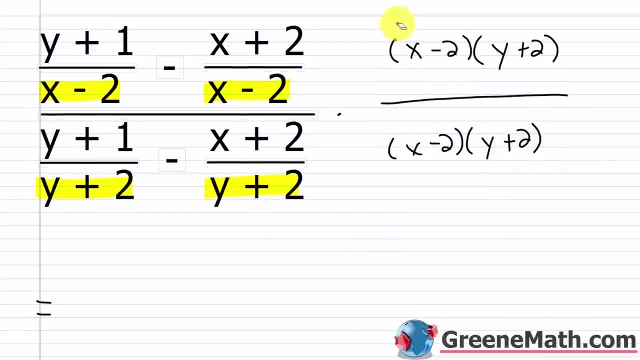 Times Y plus 2.. Now, this is pretty simple to do Because in this case, When I multiply here, In each case the X minus 2 is going to cancel And I'm just going to be left With the Y plus 2 times the numerator. 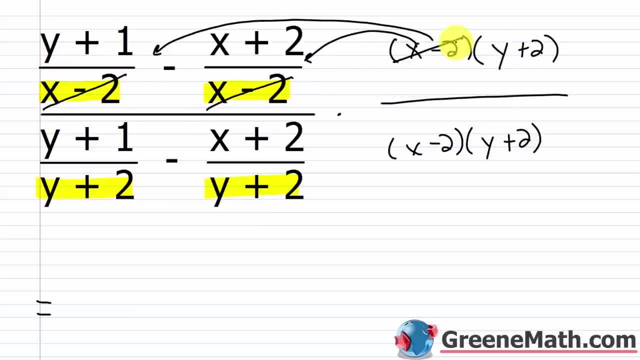 In other words, this is going to cancel With that in each case. So Y plus 2 times Y plus 1.. Let's write that out And I'm going to leave it in factored form for now, And then I'm subtracting away. 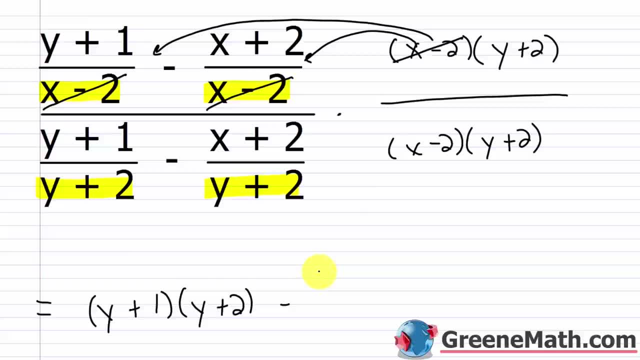 And you can put that inside of brackets, Or just remember that you're subtracting The whole thing away. You have Y plus 2.. Times X plus 2.. All right, then this is over For the next one. In a similar way, 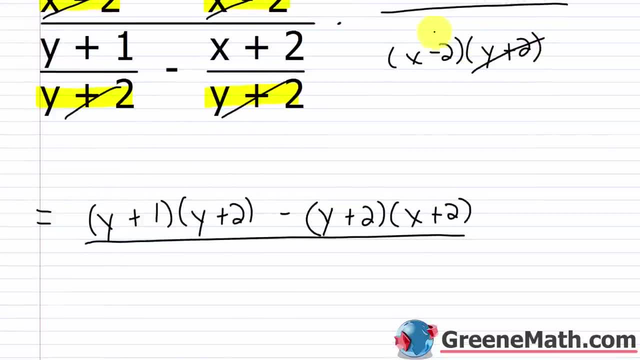 The Y plus 2 is going to cancel Here and here When I do the multiplication To each, So I'm going to be left with X minus 2.. Times Y plus 1. And then minus. In this case I'll have X plus 2.. 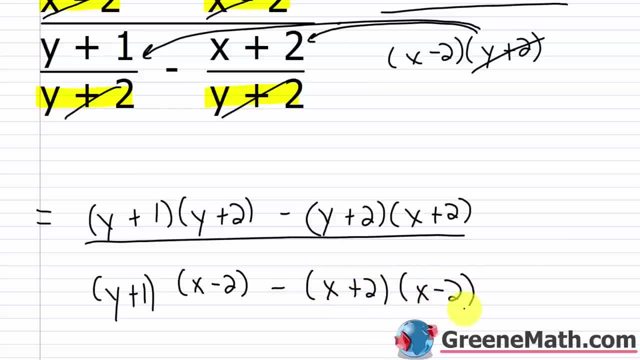 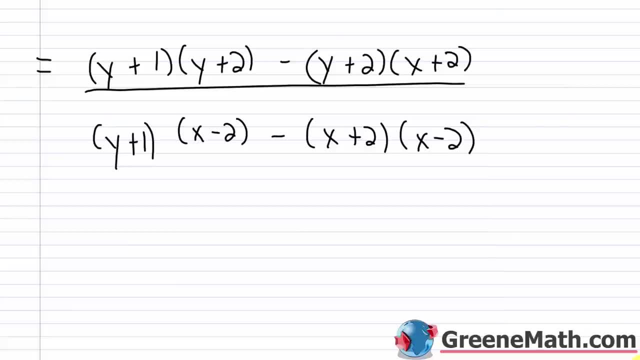 And then times X minus 2.. Okay, So now, once we get in this format, A lot of you will stop and say, Well, there's nothing I can cancel. That would be wrong. And then a lot of you will incorrectly say: 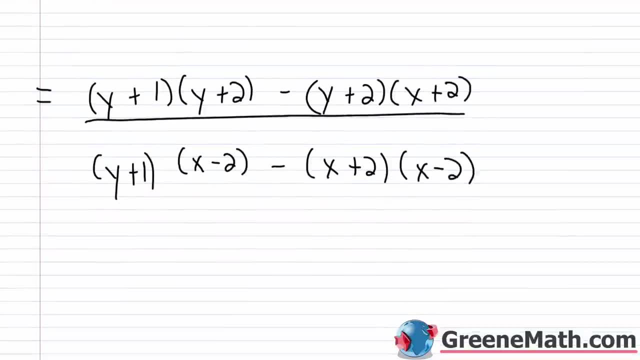 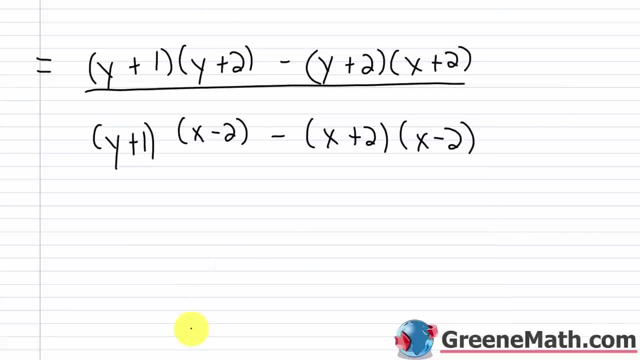 okay so now once we get in this format a lot of you will stop and say well there's nothing i can cancel that would be wrong and then a lot of you will incorrectly say well i can cancel you know between the numerator and denominator i can go this with this again you can't do that because we have subtraction 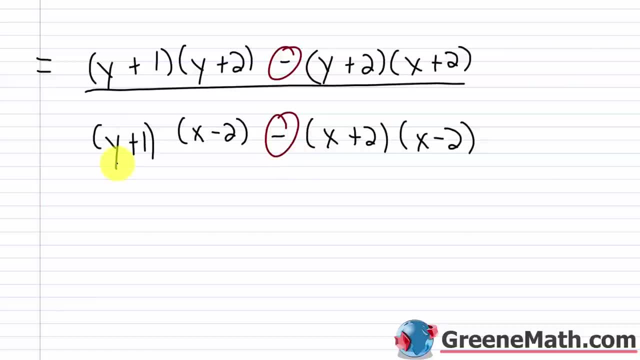 involved here if it's straight multiplication if all you have in your numerator and denominator is multiplication cancel away but if we have subtraction or addition involved you know and i know that you're seeing the subtraction here and here and the addition here and here and you're saying well how is that different it is different because these are factors right this whole thing is multiplied by this whole thing this subtraction sign 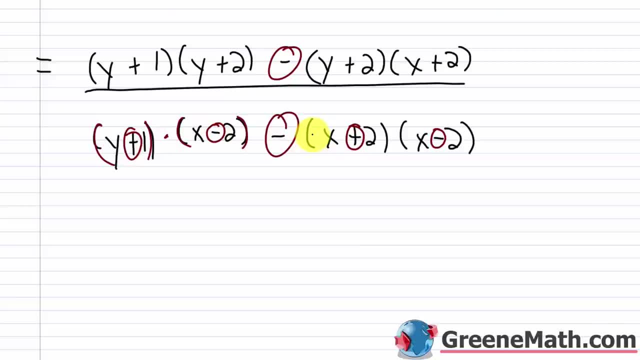 is separating these two there's no multiplication involved in that right this is a factor and this is a factor so that's how you gotta look at it and again this is one of the most common mistakes that i see and so that's why i talk about it in each and every video so that at some point you would stop and say okay i can't cancel this with this no big no no okay one of the things 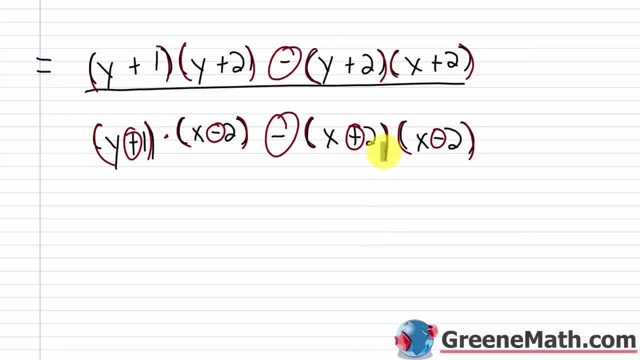 i want you to look at is that in the numerator here i have a common binomial factor of y 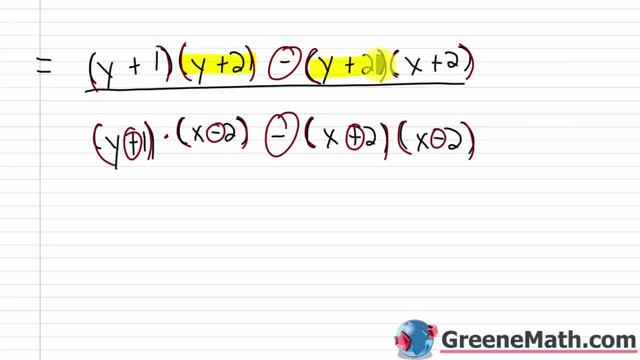 plus two in the denominator i have a common binomial factor of x minus two so what happens if we pull that out if i pulled it out so in this case i have a y plus two out in front so inside of let's say brackets i would have what's left which is y plus one that quantity minus the quantity x plus two 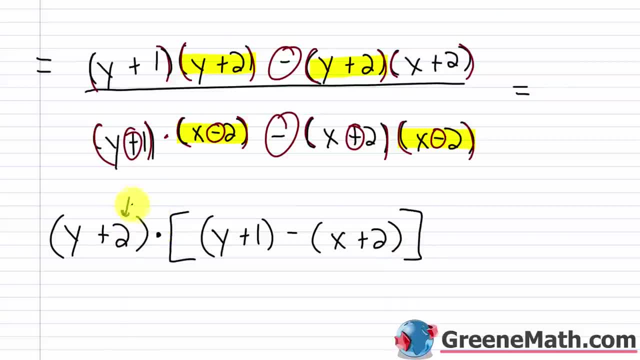 now this is multiplication this is a factor 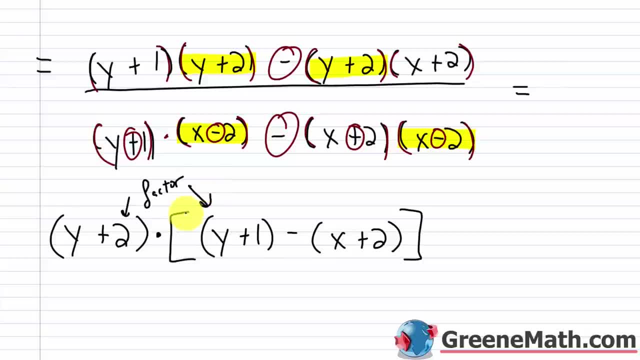 and this is a factor this whole thing here let me just highlight it the whole thing is a factor now 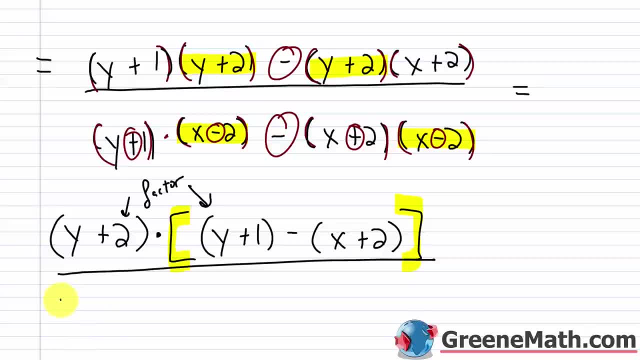 this is gonna be over if i pull out the x minus two here 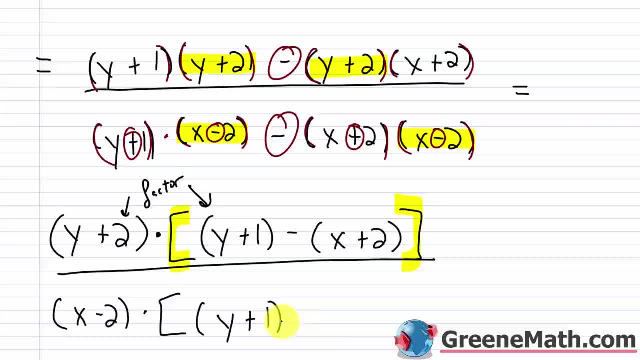 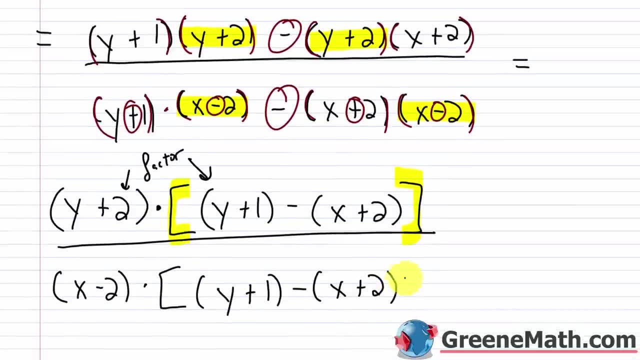 inside of brackets i'm gonna have y plus one that quantity minus over here i'd have x plus two now we can cancel between the numerator and denominator here because we are 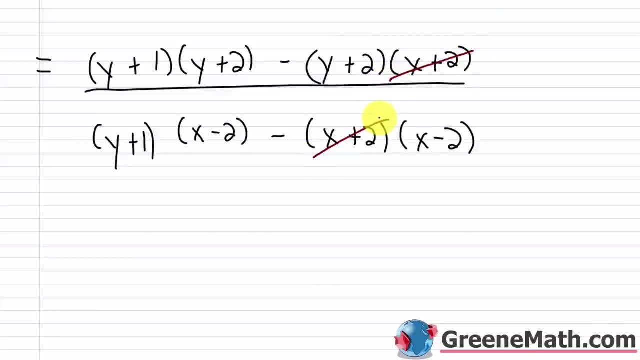 Well, I can cancel Between the numerator and denominator. I can go this with this Again. you can't do that because We have subtraction involved here. If it's straight multiplication, If all you have in your numerator and denominator Is multiplication, 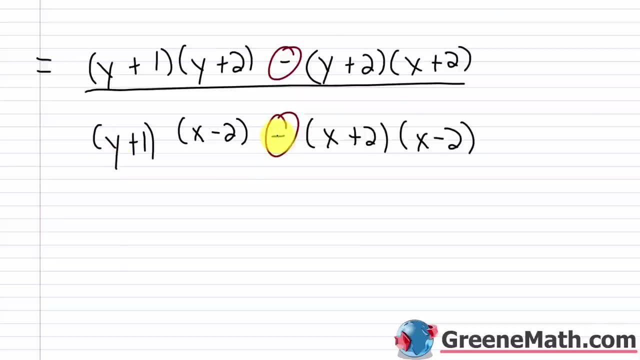 Cancel away. And I know that you're seeing The subtraction here And here and the addition here And here and you're saying: Well, how is that different? It is different because these are factors. This whole thing is multiplied by this whole thing. 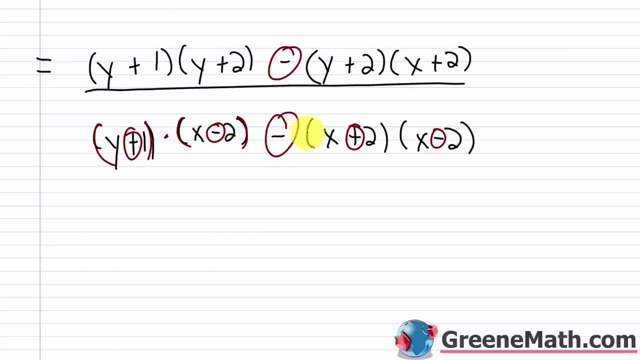 This subtraction sign Is separating these two. There's no multiplication involved in that. This is a factor, And this is a factor. So that's how you got to look at it And again, this is one of the most common mistakes that I see. 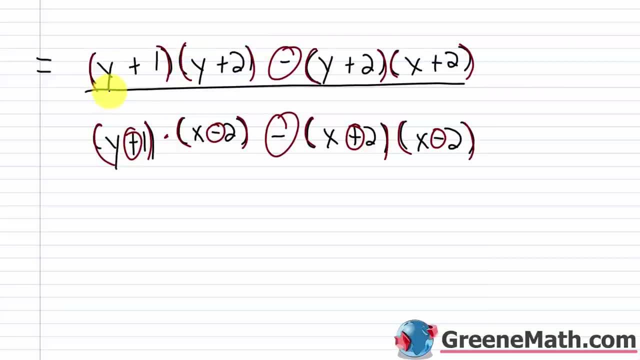 And so that's why I talk about In each and every video, So that at some point, you would stop and say, Okay, I can't cancel This with this. No big, no, no, Okay, one of the things I want you to look at: 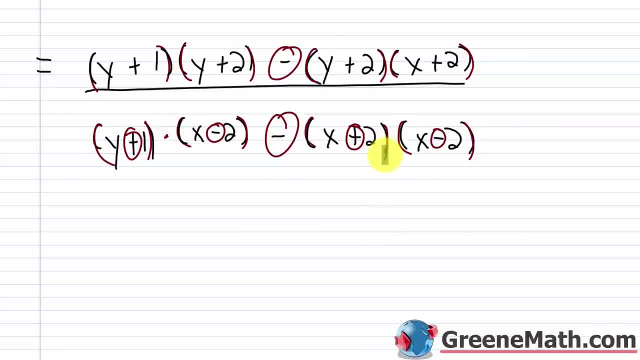 Is that in the numerator here I have a common Binomial factor of y plus two. In the denominator I have a common Binomial factor of x minus two. So what happens if we pull that out, If I pulled it out? 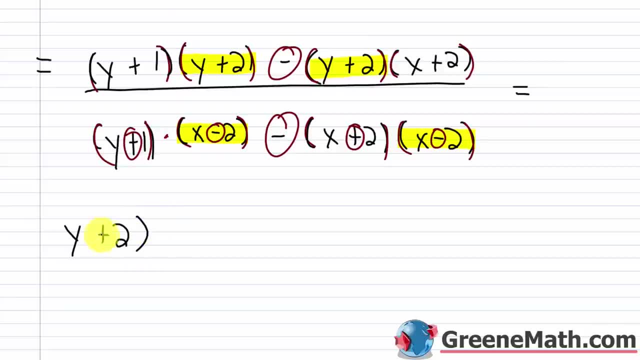 So in this case I have a common. So inside of, let's say, brackets, I would have what's left Which is y plus one, that quantity Minus the quantity x plus two. Now, this is multiplication. This is a factor. 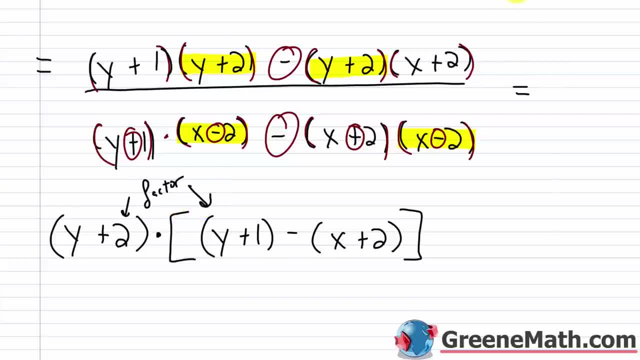 And this is a factor, This whole thing here. Let me just highlight it. The whole thing is a factor. This is going to be over. If I pull out the x minus two Here Inside of brackets, I'm going to have y plus one. 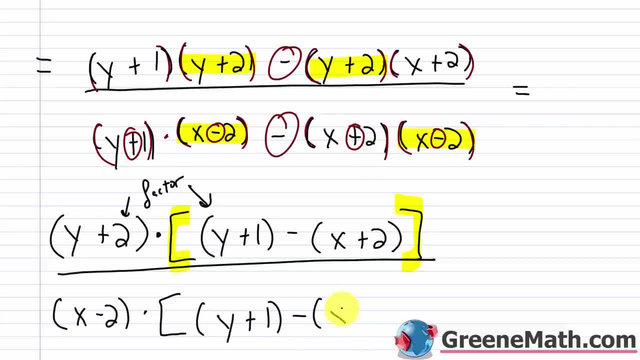 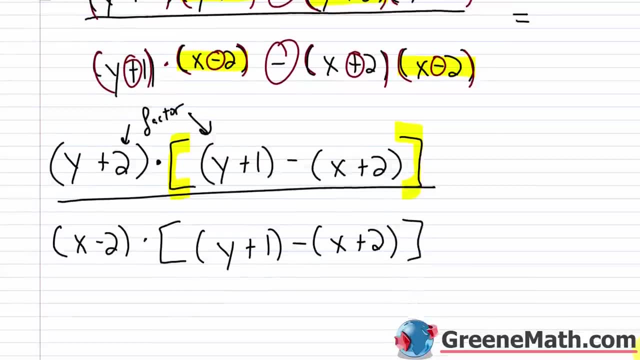 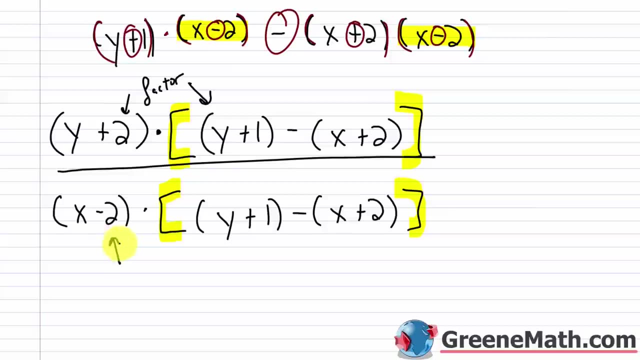 That quantity minus Over here I'd have x plus two. Now We can cancel Between the numerator and denominator here, Because we are canceling common Factors Again. let me kind of show this: This is a factor, And this is a factor. 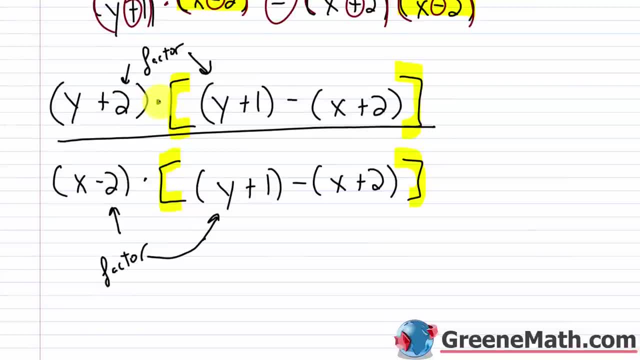 So we don't have Any subtraction here. If I had this Minus this And this plus this Or this minus this, I can't cancel, Because there is addition and subtraction involved. I don't have that. What I have is multiplication. 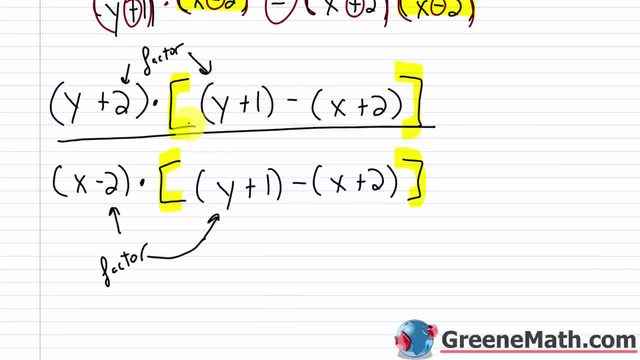 I have two factors here That are being multiplied. This is the entire factor That consists of the quantity y plus one Minus the quantity x plus two. With this factor, Again, of the quantity y plus one Minus the quantity x plus two, 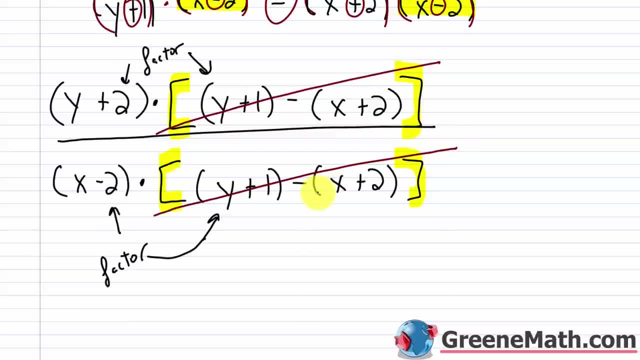 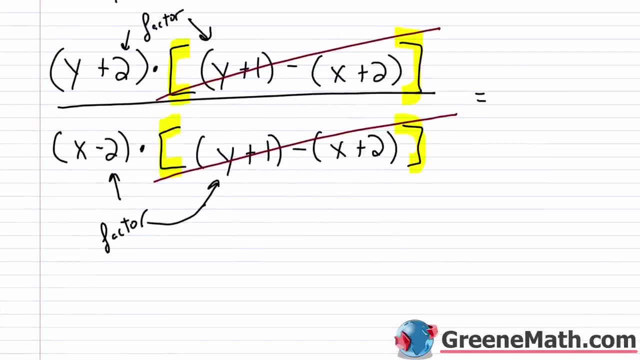 This over. this Is equal to one. They can be cancelled, So What I'm going to be left with here Once I cancel that out Is just going to be a y plus two Over an x minus two And again. 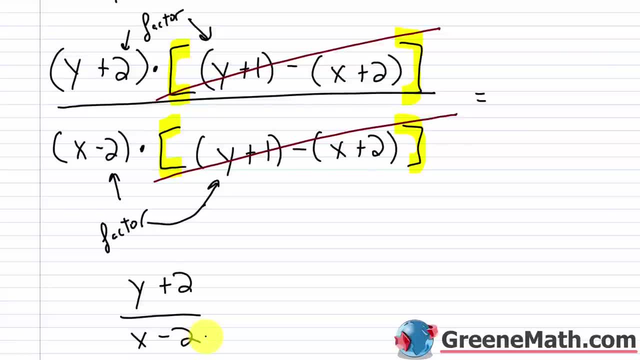 Particularly in algebra one. It's kind of the first time you're introduced to these concepts. It can be very confusing What you can cancel And what you can't Again, if you're only looking at multiplication. So in other words here: 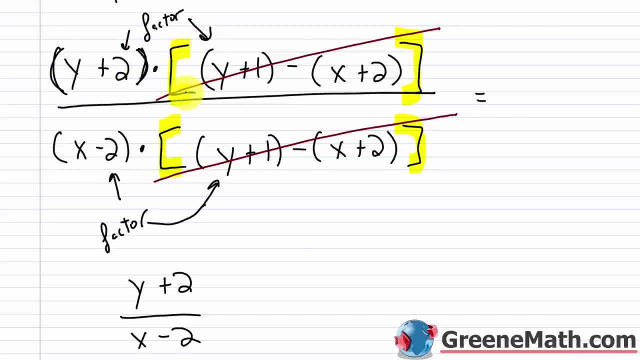 This quantity y plus two Is multiplied by this quantity, Which inside has The quantity y plus one Minus the quantity x plus two. This is multiplication. You just have factors here. Okay, You have addition and subtraction. I know that's what makes it confusing. 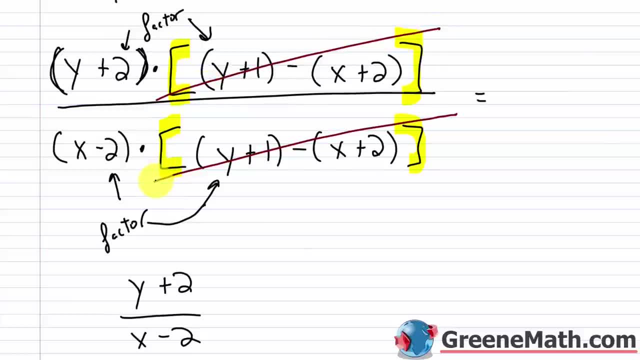 But again, again, again, This thing right here is a factor Which can be cancelled with the same factor down here. So that leaves me with what's left, Which is y plus two Over x minus two. Hello and welcome to algebra one, lesson forty eight. 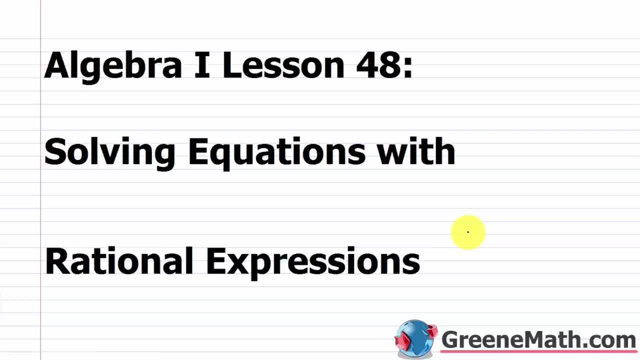 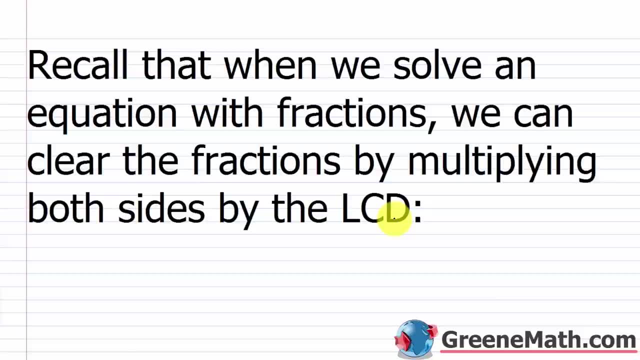 In this video We're going to learn about solving equations With rational expressions. So before we kind of jump in and start talking about Solving an equation with rational expressions, I just want to refresh everybody's memory With something that we learned. 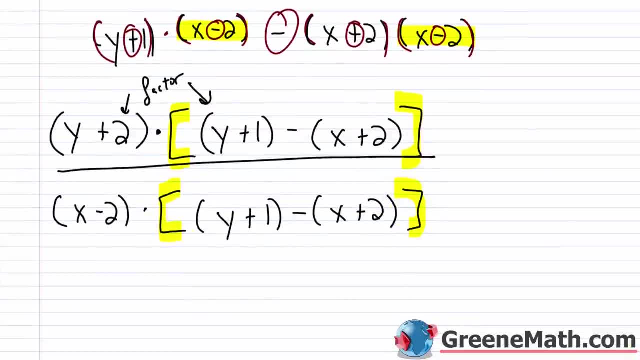 canceling common factors again let me kind of show this this is a factor and this is a factor okay 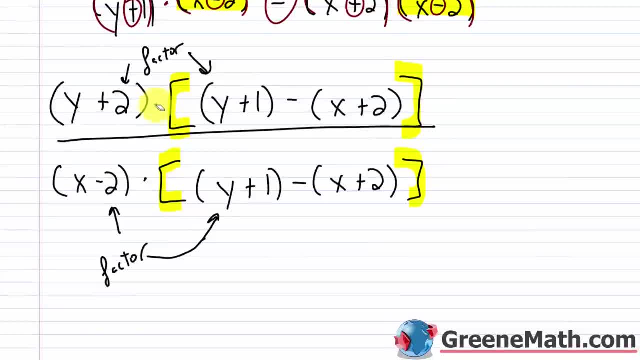 so we don't have any subtraction here if i had this minus this and this plus this or this minus this i can't cancel right because there's addition and subtraction involved 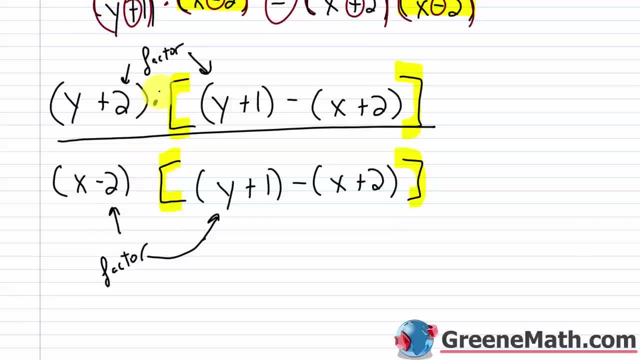 i don't have that what i have is multiplication i have two factors here that are being multiplied i have two factors here 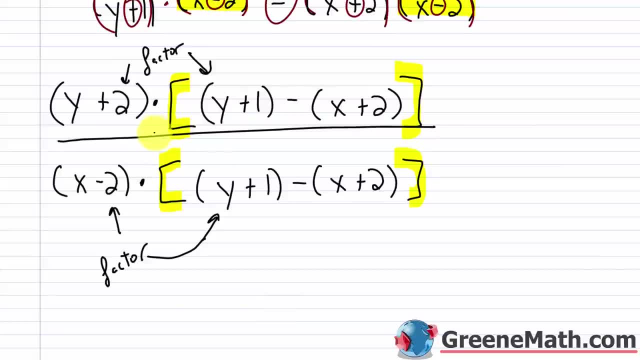 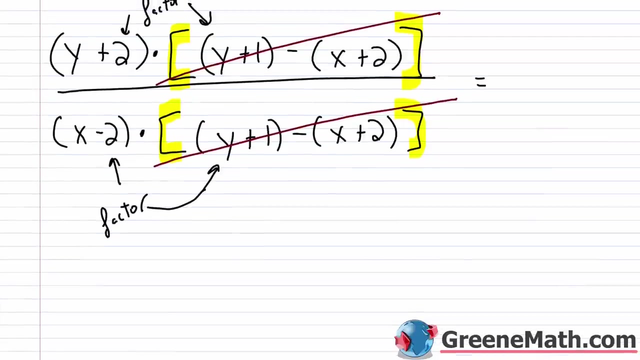 that are being multiplied so i'm gonna cancel this entire factor that consists of the quantity y plus one minus the quantity x plus two with this factor again of the quantity y plus one minus the quantity x plus two this over this is equal to one they can be cancelled so what i'm gonna be left with here once i cancel that out it's just gonna be a y plus two over an x minus two 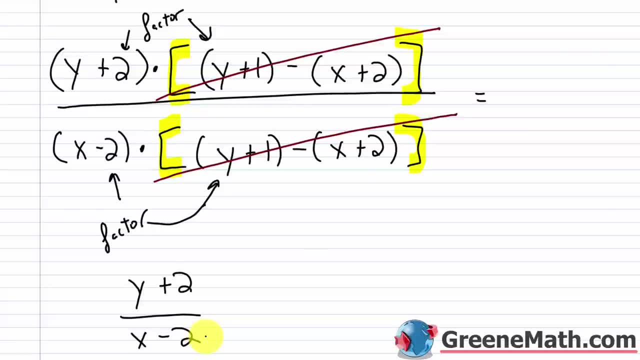 and again i know that when you first start doing this particularly in algebra one it's kind of the first time you're introduced to these concepts it can be very confusing what you can cancel and what you can't again if you're only looking at multiplication so in other words here this quantity y plus two is multiplied by this quantity which inside has the quantity y plus one minus the quantity x plus two this is multiplication you just have factors here okay same thing down 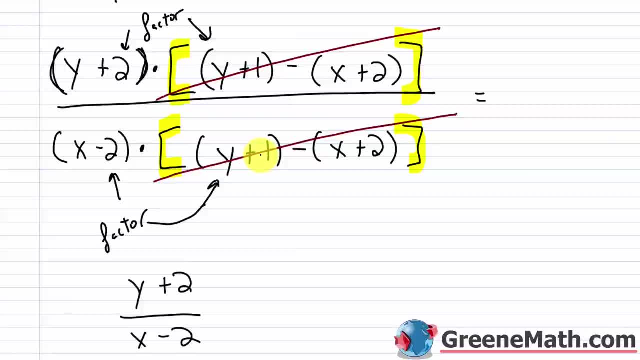 here you just have factors here now within those factors you do have addition and subtraction i know that's what makes it confusing but again again again this thing right here is a factor which can be cancelled with the same factor down here so that leaves me with what's left which is y plus 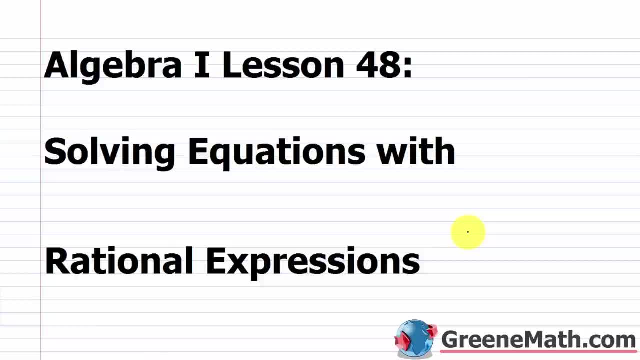 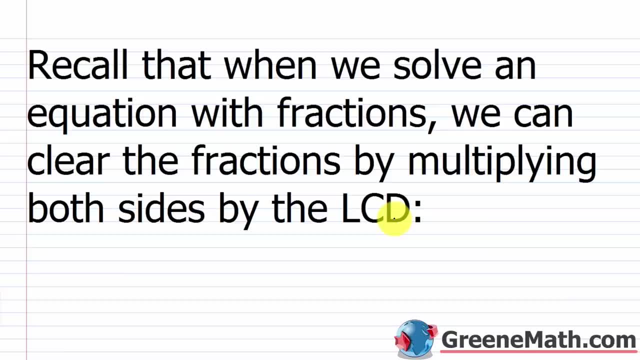 two hello and welcome to algebra one lesson forty eight in this video we're gonna learn about solving equations with rational expressions so before we kind of jump in and start talking about solving an equation 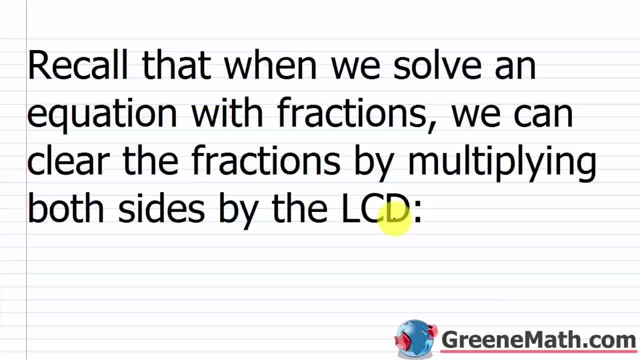 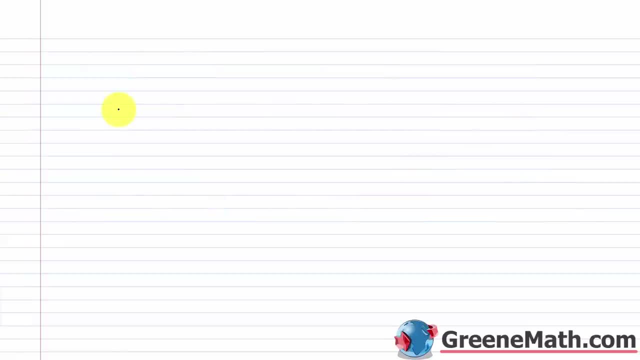 with rational expressions i just want to refresh everybody's memory with something that we learned at the very beginning of algebra one so i want you to recall that when we solve an equation with fractions we can clear the fractions by multiplying both sides by the lcd so as a quick example let's say we saw something like four fifths x plus seven thirds x and this is equal to ninety four well if i didn't want to work with the fractions of course i could 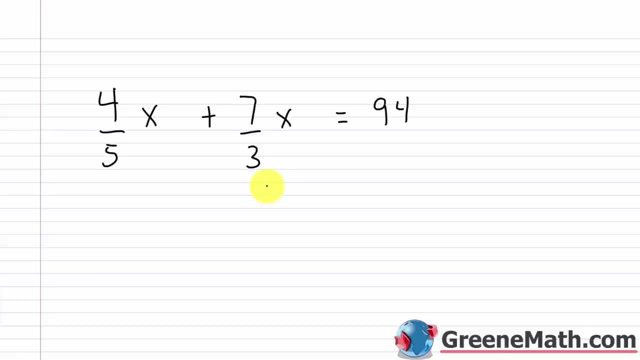 work with the fractions if i wanted to but if i didn't want to work with them i could multiply both sides of the equation by the lcd and it would clear the fractions for me so in this particular case i have a denominator of five and a denominator of three neither one of those is gonna factor so the lcd would be five times three or fifteen so i would multiply this side of the equation by fifteen and to make it legal i would multiply this side of the equation by fifteen remember your multiplication property of equality i can multiply both sides of the equation 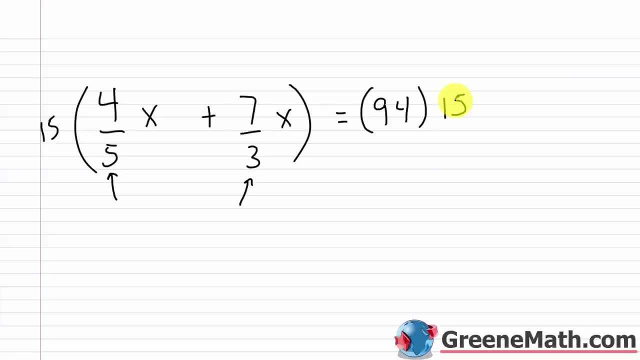 by the same non zero value and i'm not gonna change the solution so if i multiply fifteen times four fifths the fifteen would cancel with the five and give me a three three times four is twelve so this would be twelve x and then let me erase this real quick we would do that again over here so plus the fifteen would cancel with the three and give me a five five times seven is thirty five so this would be thirty five x and this equals we'd have ninety four times fifteen which would be one thousand 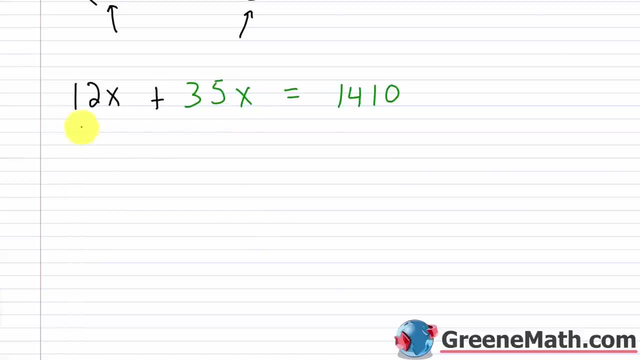 four hundred ten alright so the first thing i notice now is that i don't have any fractions anymore so now i just solve it as i normally would twelve x plus thirty five x would give me forty seven x so this is forty seven x this is equal to one thousand four hundred ten divide both sides of the equation by forty seven and i will get that x is equal to thirty 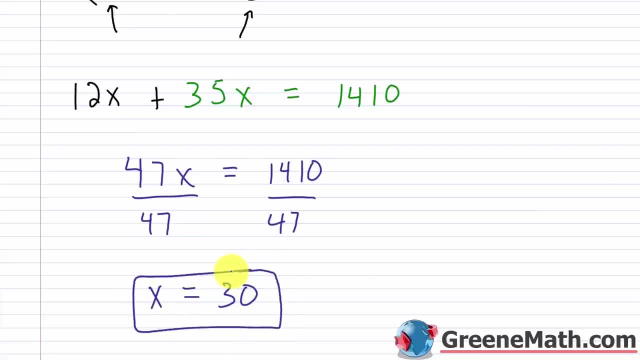 so now on almost every occasion i tell you to check the work to make sure it's accurate 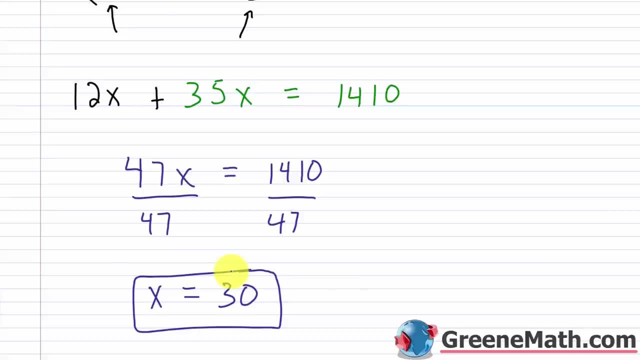 i've already checked this i know that thirty is the correct solution but if you want to you can pause the video and go ahead and check it in the interest of time i'm gonna skip that for now and just gonna kinda 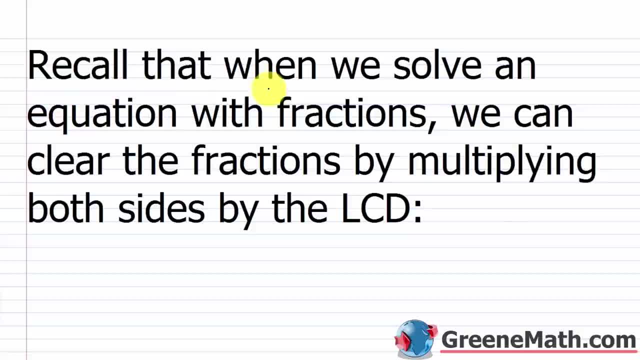 At the very beginning of algebra one. So I want you to recall That when we solve an equation with fractions, We can clear the fractions By multiplying both sides By the LCD. So as a quick example, Let's say we saw something like: 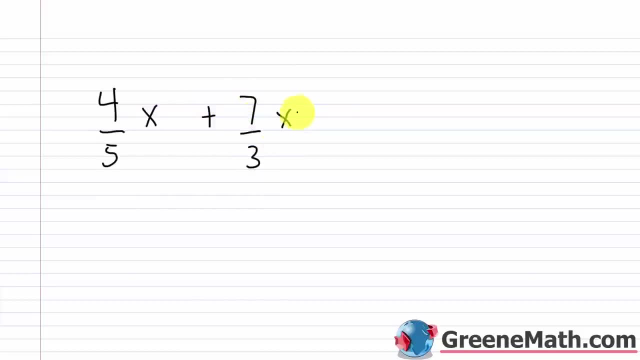 Four fifths x Plus seven thirds x, This is equal to ninety four. Well, if I didn't want to work with the fractions? Of course I could work with the fractions if I wanted to, But if I didn't want to work with them, 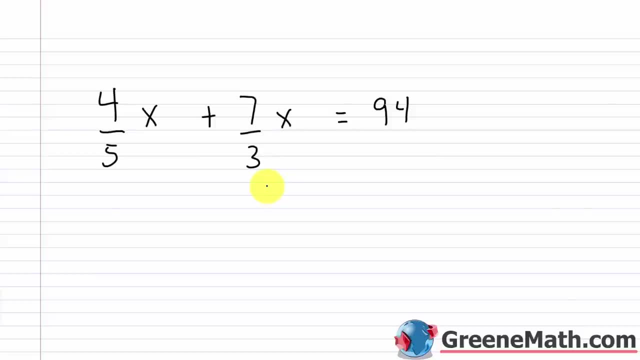 I could multiply both sides of the equation By the LCD And it would clear the fractions for me. So in this particular case I have a denominator of five And a denominator of three. Neither one of those is going to factor, So the LCD would be five times three or fifteen. 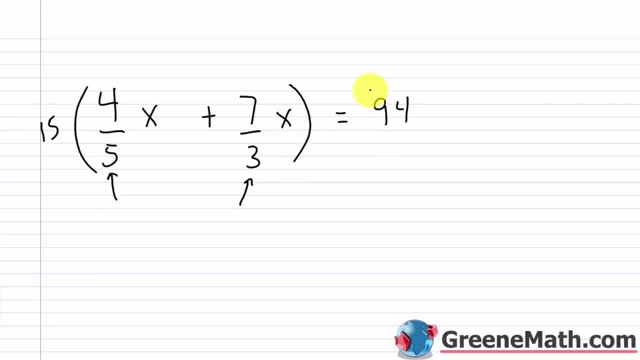 So I would multiply this side of the equation By fifteen And to make it legal, I would multiply this side of the equation by fifteen. Remember your multiplication property of equality. I can multiply both sides of the equation By the same non zero value. 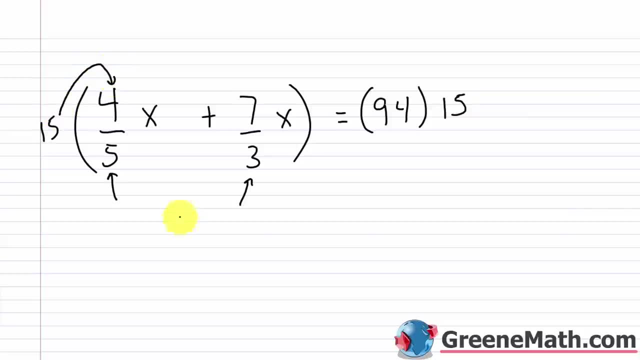 To get the solution. So if I multiply fifteen times four, fifths, The fifteen would cancel with the five And give me a three. Three times four is twelve, So this would be twelve x. And then let me erase this real quick. 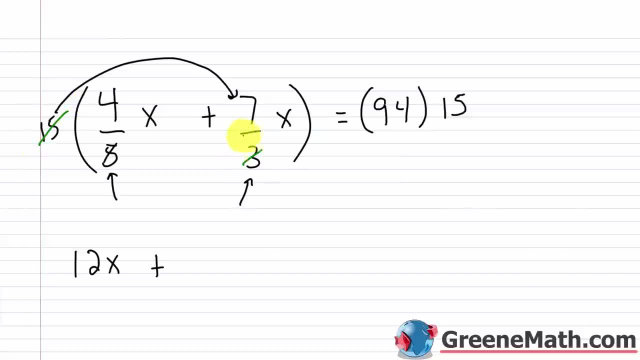 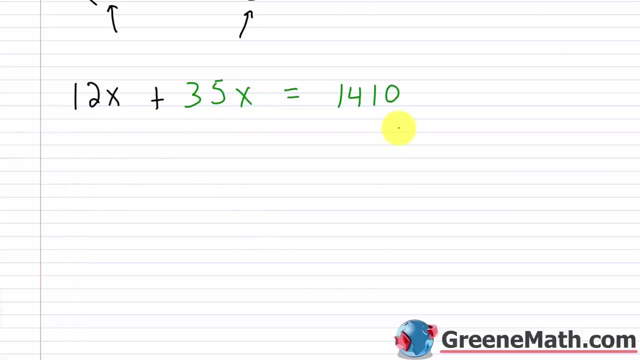 We would do that again Over here. So plus The fifteen would cancel with the three And give me a five. Five times seven is thirty five, So it would be thirty five x And this equals I don't have any fractions anymore. 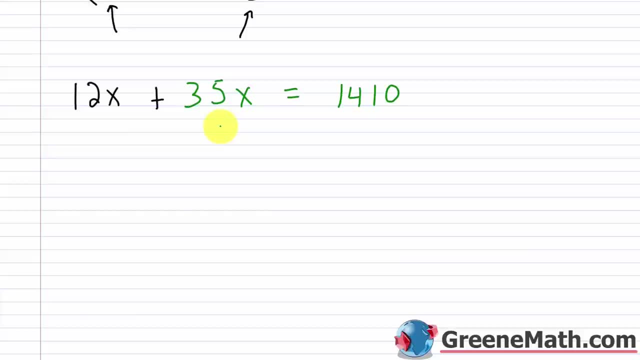 So now I just solve it as I normally would. Twelve x plus thirty five x Would give me forty seven x. So this is forty seven x. This is equal to one thousand four hundred ten. Divide both sides of the equation By forty seven. 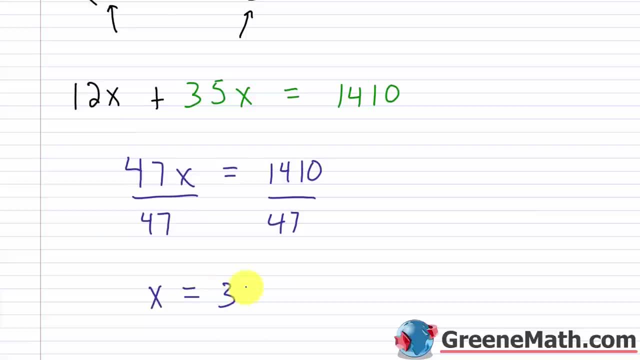 And I will get that x is equal to Thirty. Now, on almost every occasion, I tell you to check the work To make sure it's accurate. I've already checked this, But if you want to, You can pause the video. 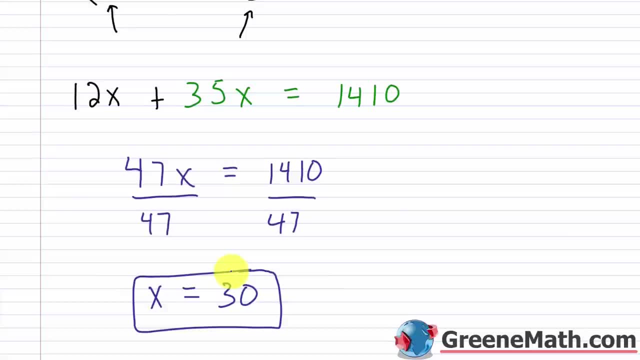 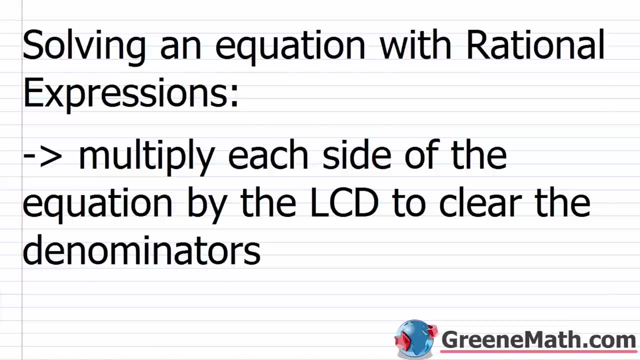 And go ahead and check it. In the interest of time, I'm going to skip that for now And just kind of get to the main content of the video. Alright, so now we want to talk about Solving an equation with rational expressions. 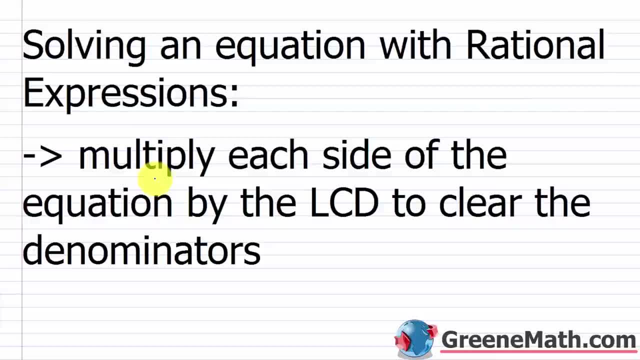 And the reason I gave you that example Is because we're going to use a similar technique here. I want you to multiply each side of the equation By the LCD. The LCD to clear the denominators. Okay, Just like we did in the previous example. 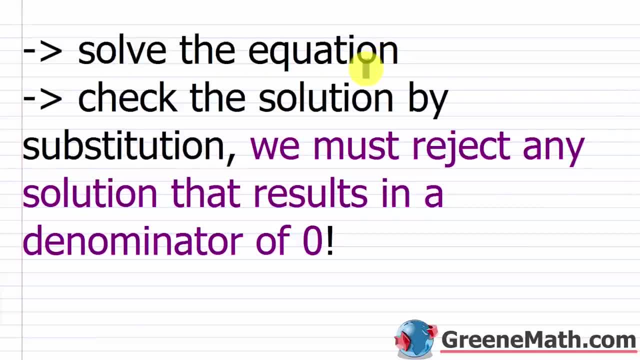 The next thing you're going to do Is you're going to solve the equation And then we're going to check the solution by substitution, Just like I always tell you to do. But here's the key thing With a rational expression. 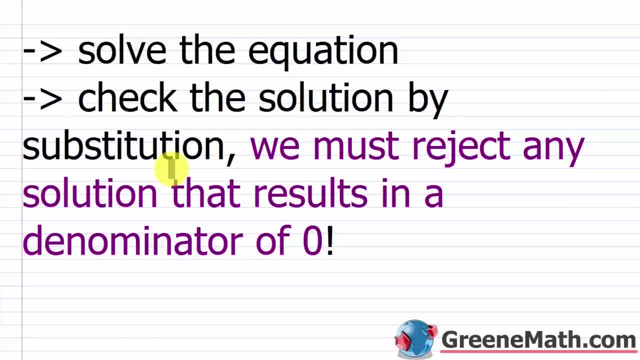 When you have variables in your denominator. Remember We cannot divide by zero. So I have this statement here: We must reject any solution That results in a denominator of zero. Very, very important That you understand that. If you want to look at the denominators, 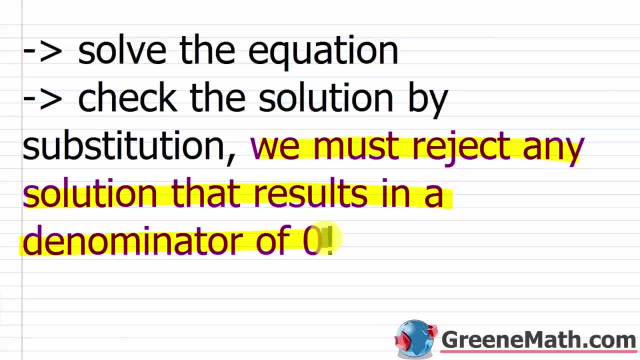 Before you kind of get going and say, Hey, these are the restricted values, Do that That way, if you get that as an answer, You can just reject it immediately. Or if you want to go back and plug in, See what results in zero. 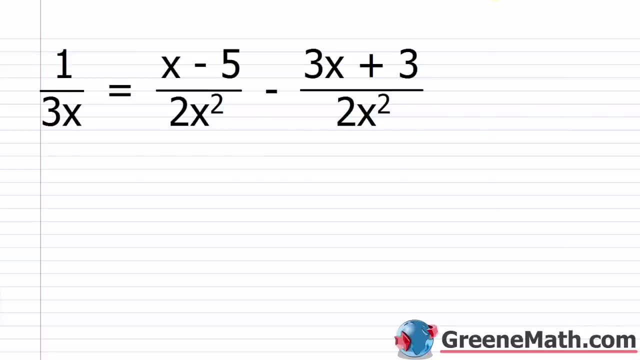 After you've done the problem, That's fine too, Alright. so let's take a look at the first example. here We have one over three x, And this is equal to X minus five over two x squared. And then minus three x plus three over two x squared. 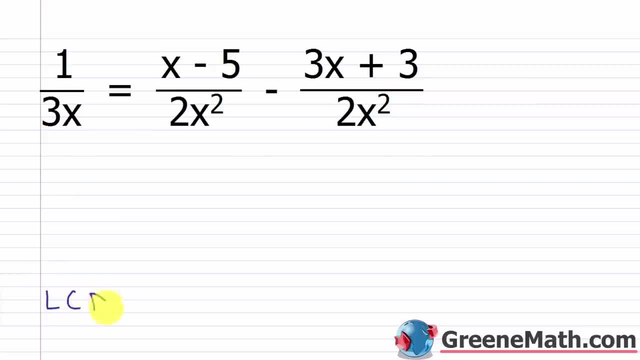 So what I'm going to do Is I'm going to figure out what the LCD is. Okay, what is my LCD? So in this particular case, I have a denominator that's two x squared, Two x squared And three x. So if I break this down, 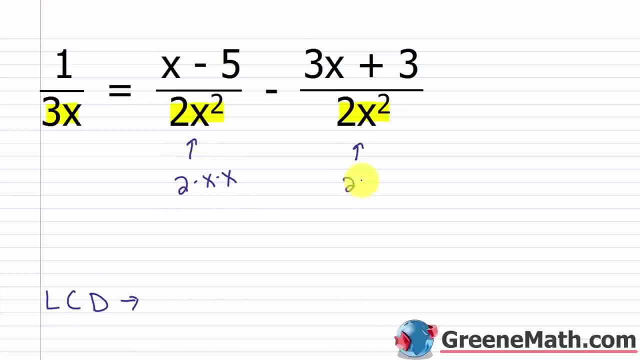 I know this is two times x times x. I know this is two times x times x, And I know this is three times x. So again, We know how to get an LCD at this point. We've watched several videos where we've done this. 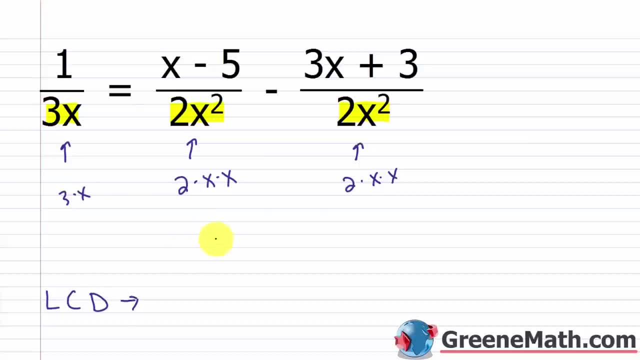 And essentially All I'm going to do is look for The largest number of repeats For any duplicate factor. Everything else just goes in. So for x, Because it appears in everything, I just go with the highest exponent, Which is x squared. 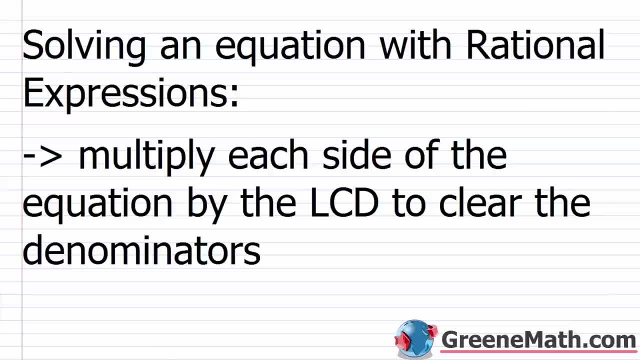 get to the main content of the video alright so now we wanna talk about 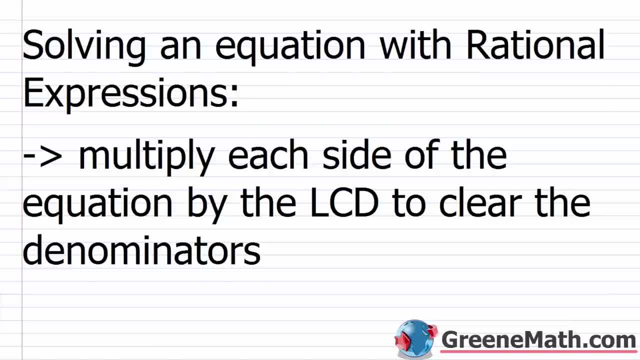 solving an equation with rational expressions and the reason i gave you that example is because we're gonna use a similar technique here i want you to multiply each side of the equation by the LCD the LCD to clear the denominators okay so we're 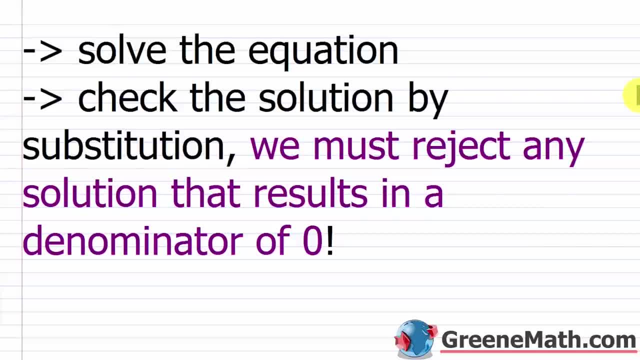 gonna do that in this case just like we did in the previous example the next thing you're gonna do is you're gonna solve the equation and then we're gonna check the solution by substitution just like i always tell you to do but here's the key thing with a rational expression when you have variables in your denominator remember we cannot divide by zero so i have this statement here we must reject any solution that results in a denominator of zero very very important that you 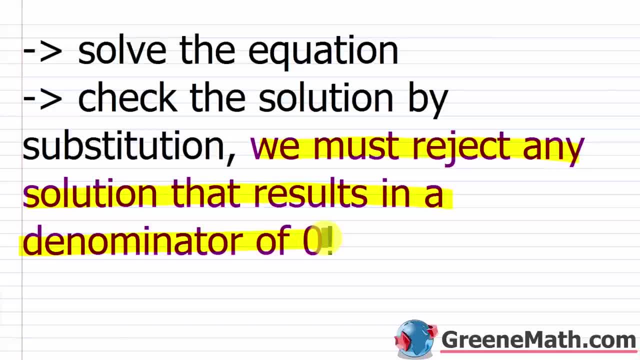 understand that okay if you wanna look at the denominators before you kinda get going and say hey these are the restricted values do that that way if you get that as an answer you can just reject it immediately or if you wanna go back and plug in see what results in zero after you've done the problem that's fine too alright so let's take a look at the first example 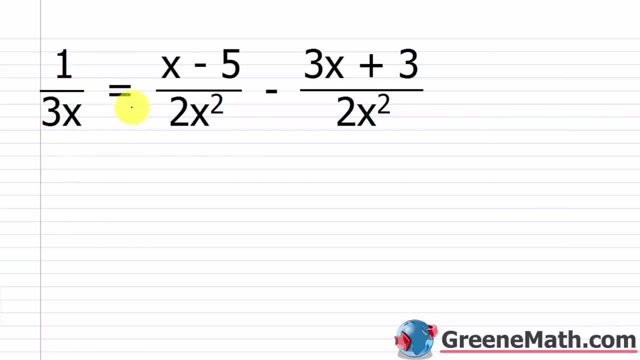 here we have one over three x and this is equal to x minus five over two x squared and then minus three x plus three over two x squared 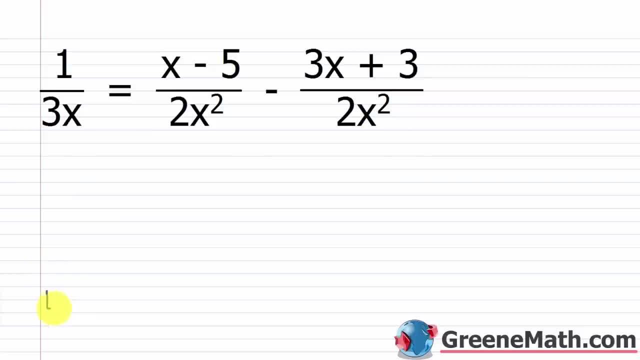 so the first thing i'm gonna do is i'm gonna figure out what the lcd is okay what is my lcd so in this particular case i have a denominator that's two x squared two x squared and three x so if i break this down i know this is two times x times x i know this is two times x times x and i know this is three times x so again we know how to get an lcd at this point we've watched several videos where we've done this 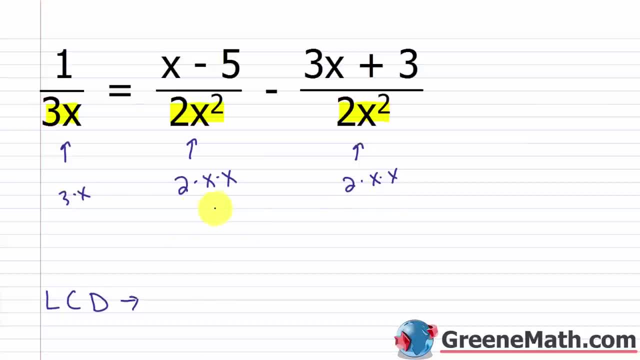 and essentially all i'm gonna do is look for the largest number of repeats for any duplicate factor everything else just goes in so for x because it appears in everything i just go with the highest exponent which is x squared then for the number parts i have a two here and a two here it only occurs once in each so that's gonna go in there and then i have a three here it only occurs one time there so i'm gonna throw that in there so i would have three times two x squared or what we'd say is six 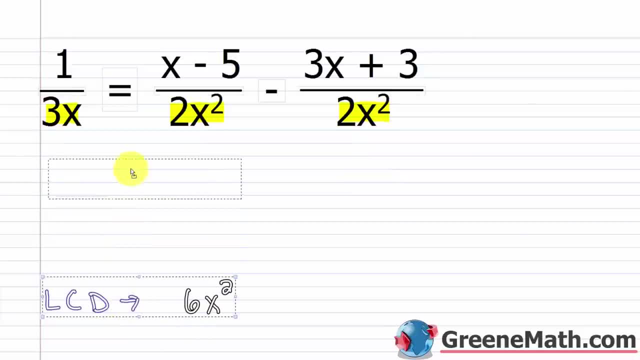 x squared for my lcd okay let me move this up here so the next thing that i wanna do i wanna multiply both sides of the equation by the lcd so i'm gonna have one over three x and i'm gonna multiply this by six x squared and this is equal to i'm gonna put parentheses around this x minus five over two x squared minus three x plus three again over two x squared and i'm multiplying this guy by 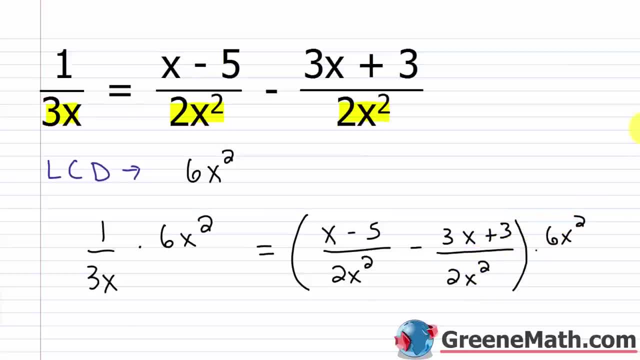 six x squared so let me scroll down and get a little room 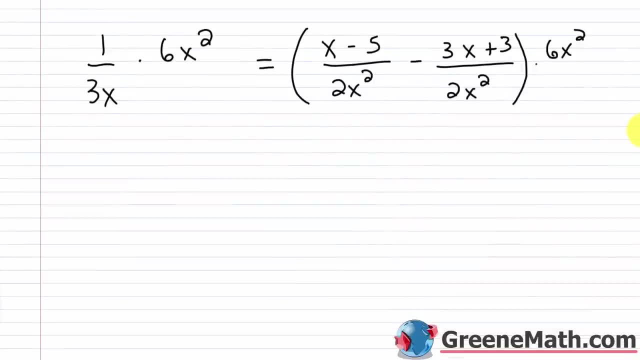 we'll come back up to the original equation in a little while 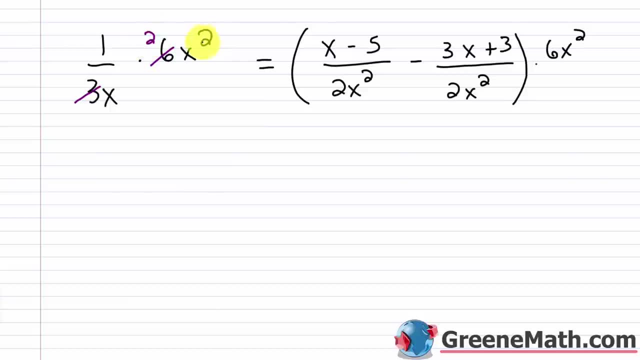 so for this one over here it's easy to see i can cancel this six with this three and get a two i can cancel one factor of x up here with this x here and so what i'm gonna be left with is just a two x right here and this is gonna be equal to i'm gonna use my distributive property here over two x squared the six would cancel with the two and give me a three and the x squareds would cancel 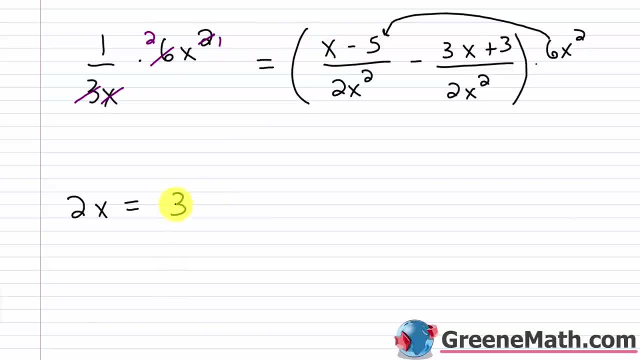 so essentially i would have three times this quantity x minus five so three times the quantity x minus five and then minus i'm gonna have six x squared times this guy right here again it's gonna be the same thing the x squareds are gonna cancel and six over two is three so i'm gonna have three times the quantity three x plus three 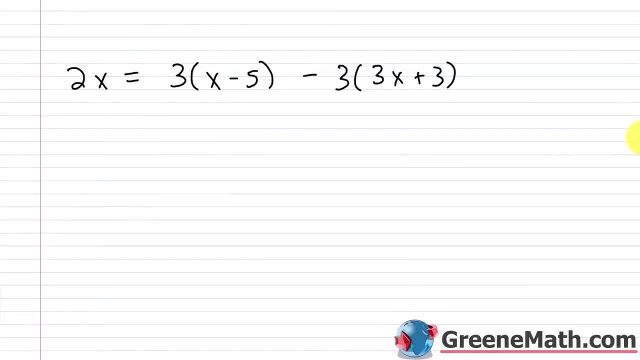 okay so moving on now i just wanna do some simplifications i have two x is equal to three times x is three x three times negative five is minus fifteen 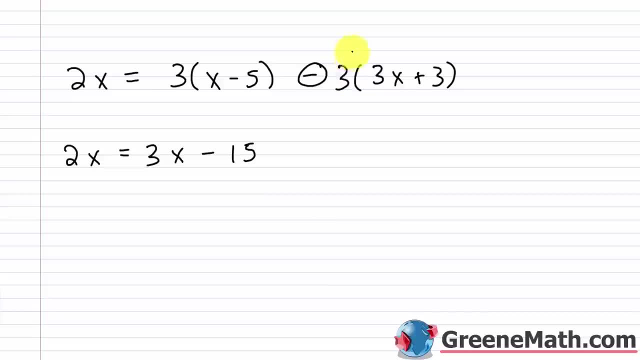 now i have a negative three here okay so pay close attention i'm gonna distribute the negative and the three to everything so negative three times three x is negative nine x 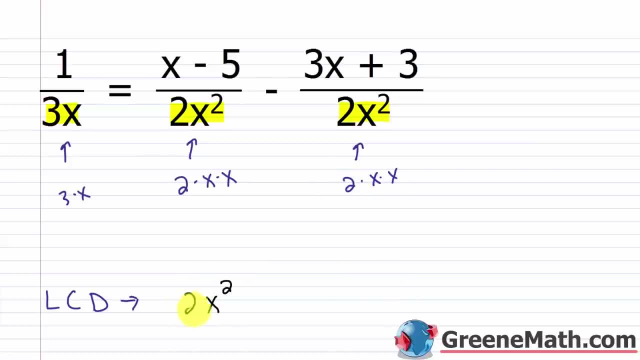 Then for the number parts, I have a two here And a two here. It only occurs once in each, So that's going to go in there. And then I have a three here, Which I'm going to say is six x squared. 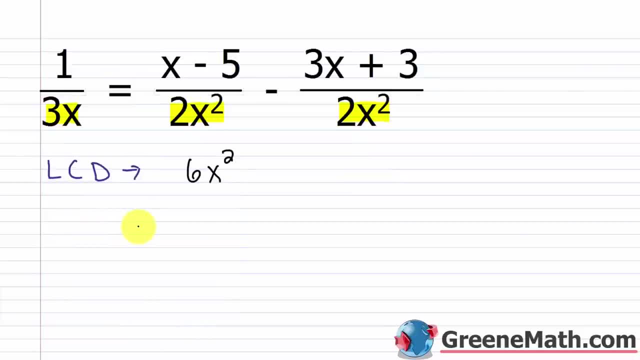 For my LCD. Okay, let me move this up here. So the next thing that I want to do, I want to multiply both sides of the equation By the LCD. So I'm going to have one over three x And I'm going to multiply this by six x squared. 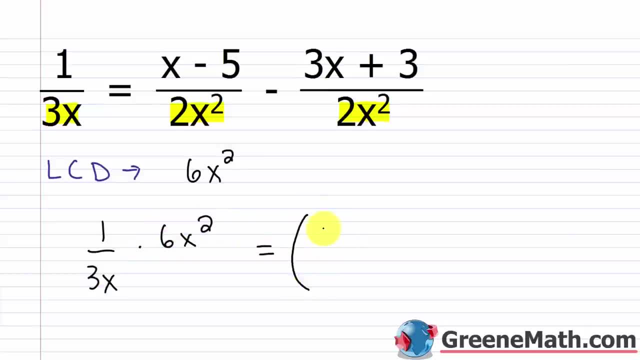 And this is equal to- I'm going to put parentheses around this- X minus five Over two x squared, Minus three x plus three, Again over two x squared, And I'm multiplying This guy by six x squared. So let me scroll down. 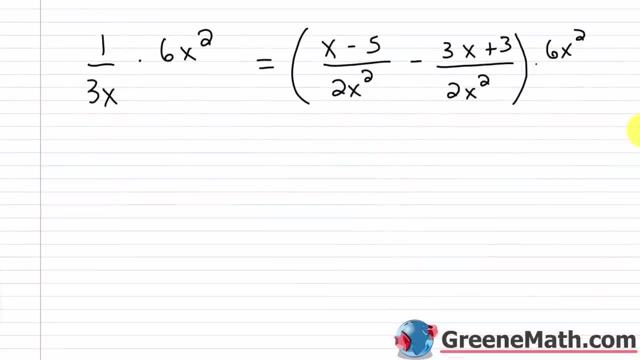 And get a little room. We'll come back up to the original equation in a little while. So for this one over here It's easy to see. I can cancel this six with this three And get a two. I can cancel one factor of x up here. 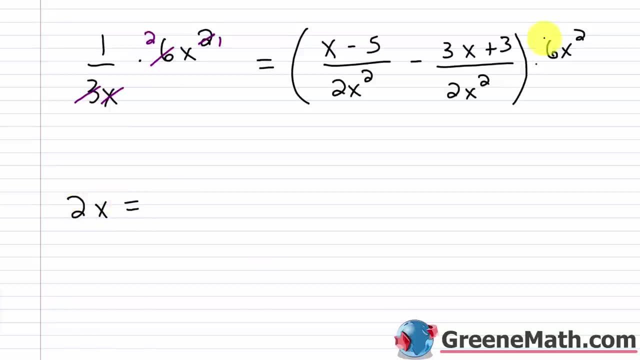 With this x here, And so what I'm going to be left with Is just a two x right here, And this is going to be equal to- I'm going to use my distributive property here- Six x squared over two x squared. 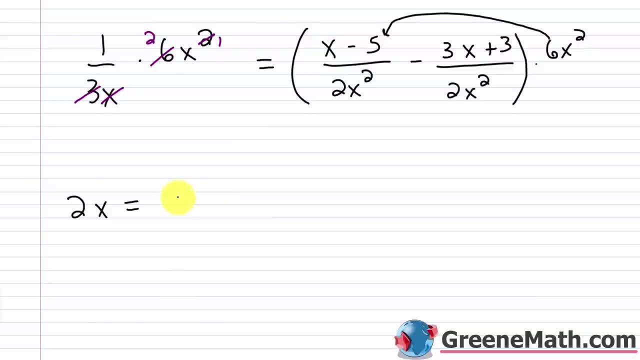 And this would cancel. So essentially I would have three times this quantity X minus five, So three times the quantity x minus five And then minus, I'm going to have six x squared times this guy right here. Again, it's going to be the same thing. 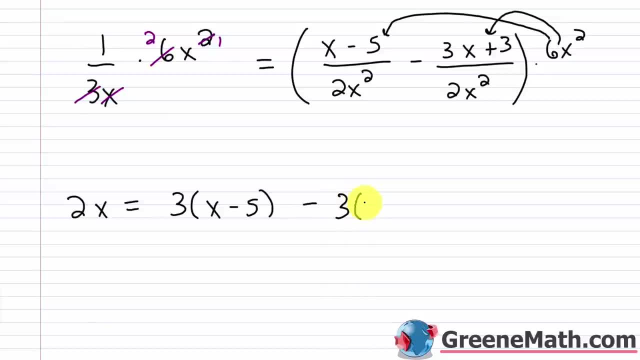 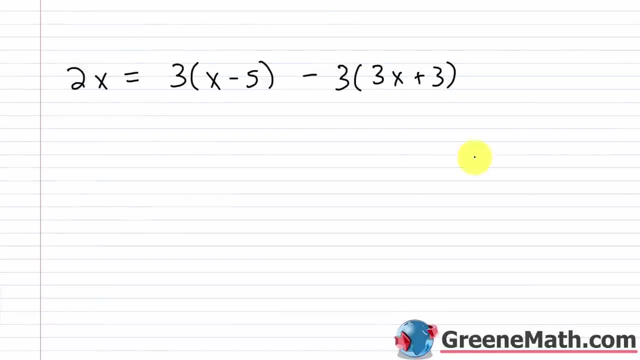 The x squared's are going to cancel, And six over two is three, So I'm going to have three times the quantity Three x plus three. Okay, so moving on now. I just want to do some simplification. I have two. x is equal to. 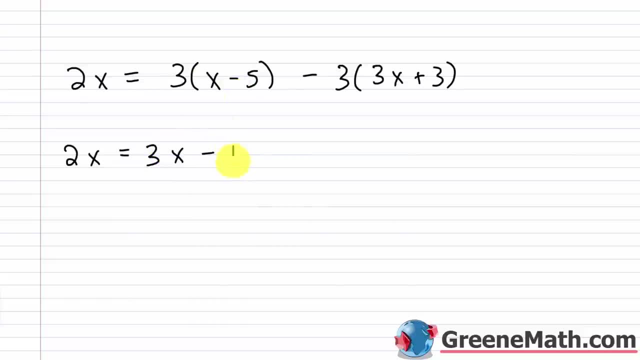 Three times x is three x. Three times negative five is minus fifteen. Now I have a negative three here. Okay, so pay close attention. I'm going to distribute the negative And the three to everything. So negative three Times three x is negative nine x. 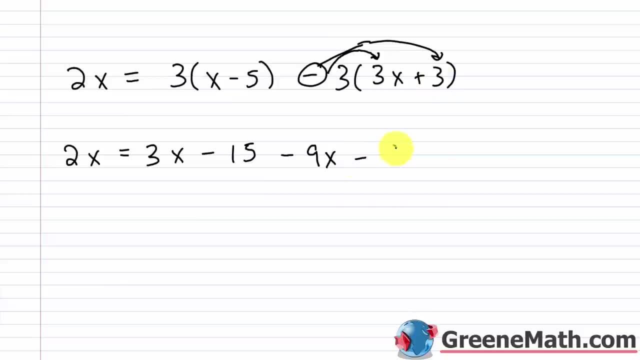 Negative three Times three is negative nine. So let's simplify. now I've got my two: x is equal to Three. x minus nine, x is negative six, x Negative. fifteen minus nine Is going to give me negative twenty four. And then 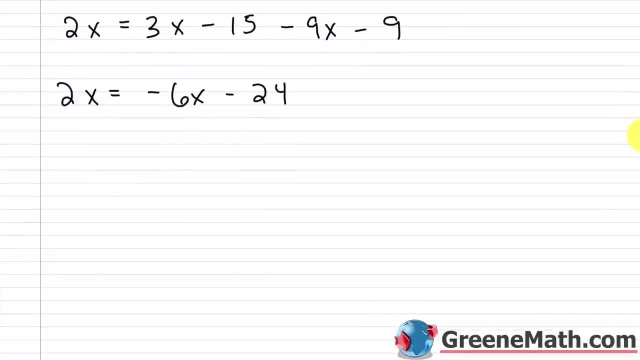 And now What I want to do is get all the x's on one side And the numbers on the other, Just like we've been doing since we started. So I'm going to add six x to both sides of the equation. So I'm going to have two x plus six x. 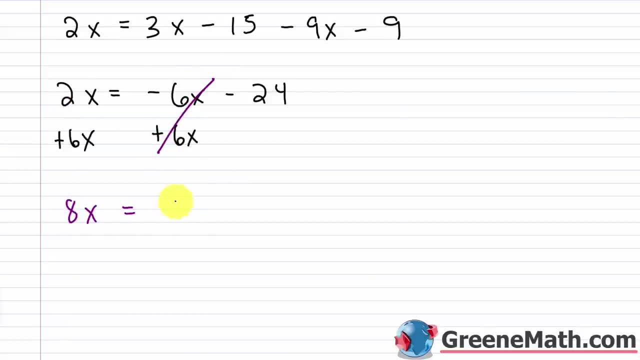 Which is eight x. This is going to cancel, And this is equal to Negative twenty four. We can then divide both sides of the equation by eight, And we're going to see that x is equal to Negative three. So let me erase everything. 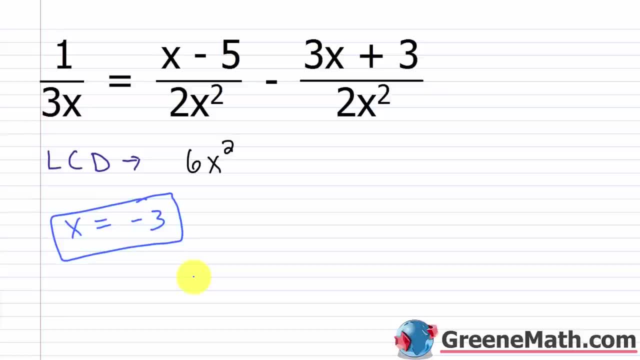 And go back up to the top, And I'm going to check to see if this is a valid solution. Okay, so what I'm going to do is plug in a negative three For each x, And so I would have one over Three times negative three. 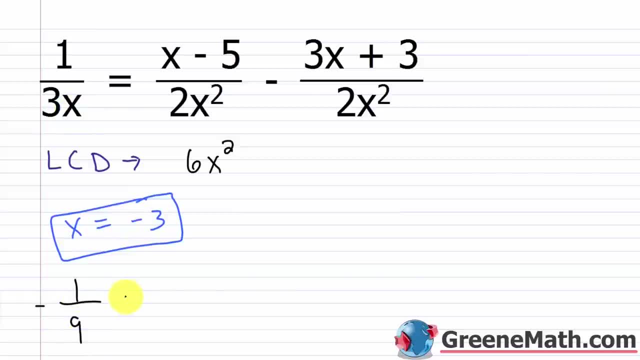 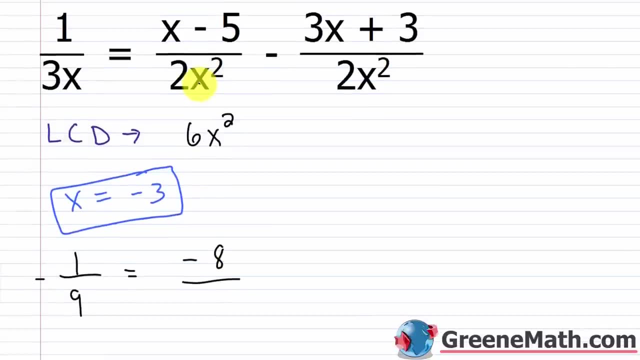 Which would be negative nine. We can go ahead and just do that. We'll put negative one ninth. This is equal to Plug in a negative three here. So negative three minus five would be negative eight Over Plug in a negative three there. 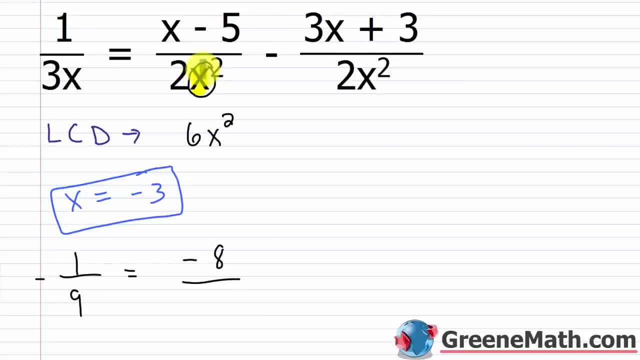 Now it's going to be squared Negative three. squared is nine Nine times two is then eighteen. So I'm going to put eighteen here And then minus Three times negative. three is negative nine. Negative nine plus three Is negative six. 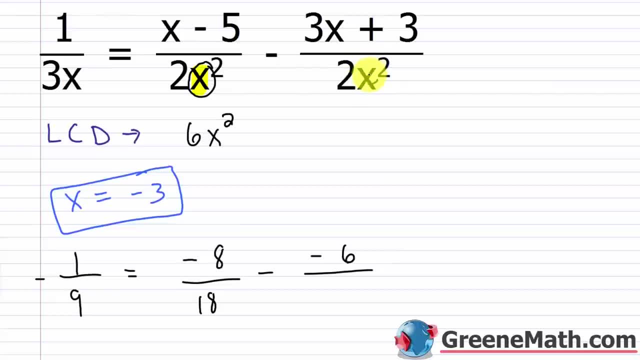 And then over Again. same thing here: If I take negative three and I square it, I get nine. Then nine times two is eighteen. So I have minus a negative, That's plus a positive. So that's the only thing I want to do there. 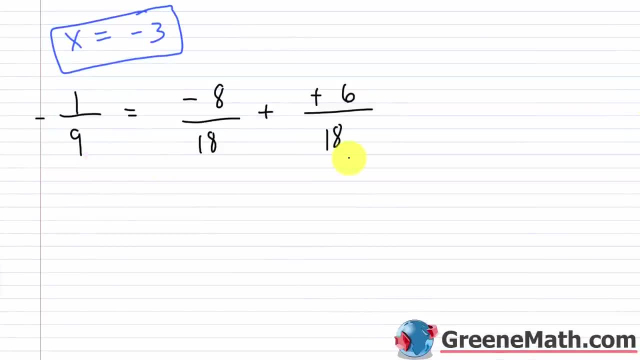 So I want to just check this. now. I see that plugging in a negative three Did not give me a denominator of zero, So we're good to go there. Now we're just checking to see if the left and the right side are equal. 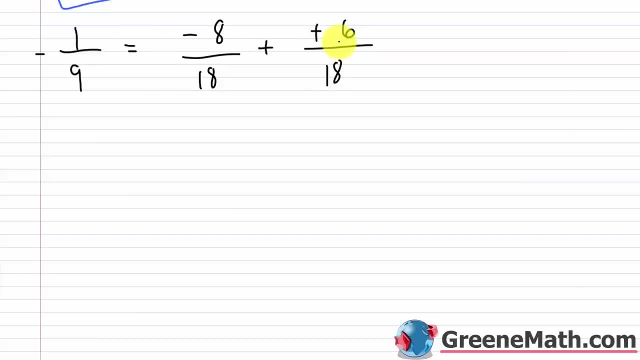 So negative eight plus six Is going to give me negative two. So this would be negative two over eighteen. So I get negative one ninth Is equal to negative two over eighteen And this would be negative one ninth If I simplify and divide numerator and denominator. 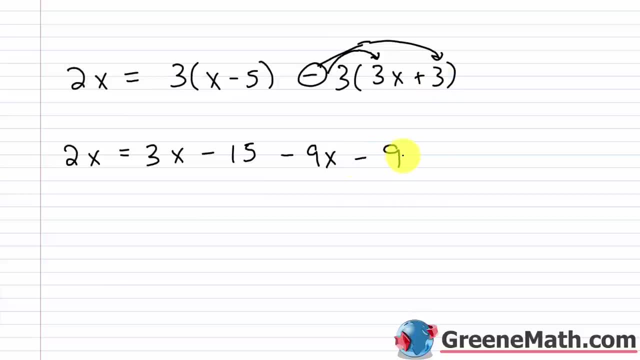 negative three times three is negative nine so let's simplify now 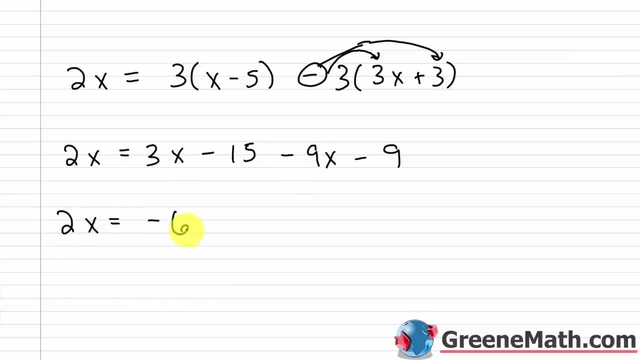 i've got my two x is equal to three x minus nine x is negative six x negative fifteen minus nine is gonna give me negative twenty four and now what i wanna do is get all the x's on one side 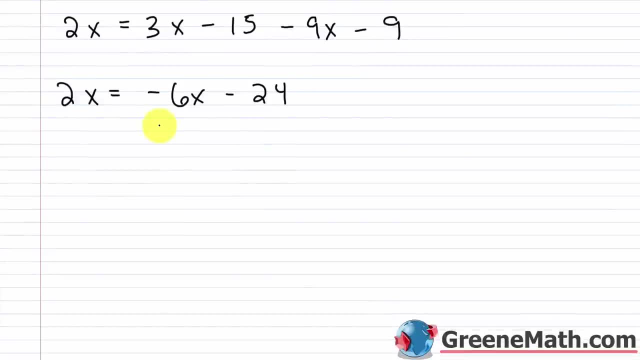 and the numbers on the other just like we've been doing since we started so i'm gonna add six x to both sides of the equation so i'm gonna have two x plus six x which is eight x this is gonna cancel and this is equal to negative twenty four we can then divide both sides of the equation by eight and we're gonna see that x is equal to negative three so let me erase everything and i'm gonna drag this answer back up to the top and i'm gonna check to see if this is a valid solution okay so what i'm gonna do is plug in a negative three 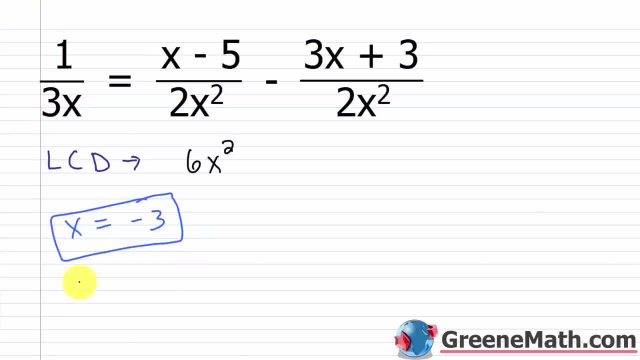 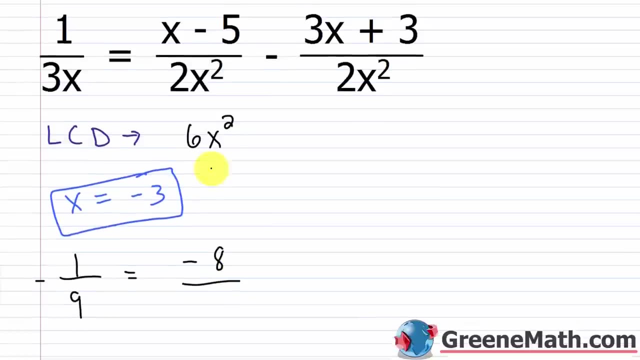 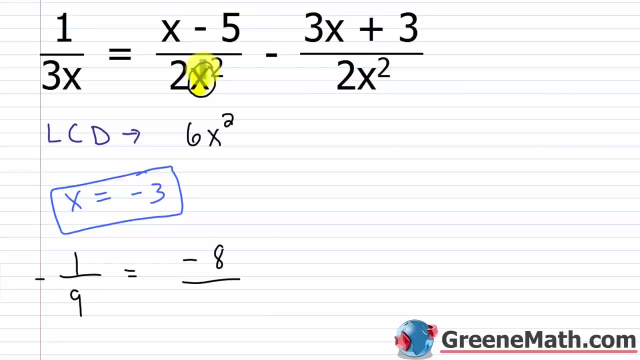 for each x and so i would have one over three times negative three which would be negative nine we can go ahead and just do that we'll put negative one ninth this is equal to plug in a negative three here so negative three minus five would be negative eight over plug in a negative three there now it's going to be squared for x so negative three the negative and the three squared is nine nine times two is then eighteen so i'm gonna put eighteen 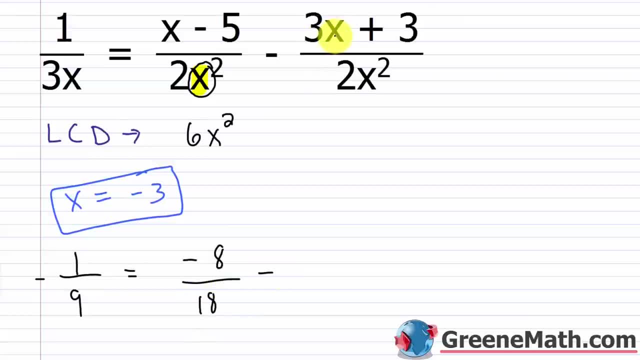 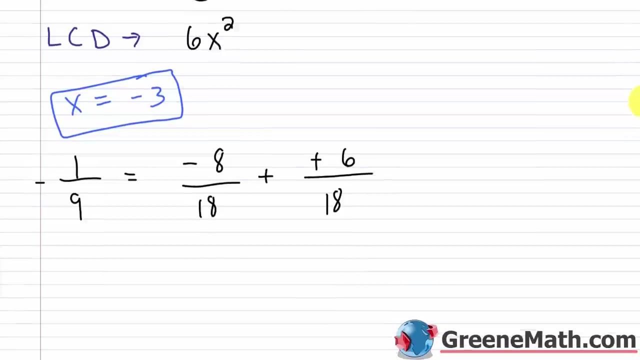 here and then minus three times negative three is negative nine negative nine plus three is negative six and then over again same thing here if i take negative three and i square it i get nine then nine times two is eighteen so i have minus a negative that's plus a positive so that's the only thing i want to do there and so i want to just check this now i see that plugging in a negative three did not give me a denominator of zero 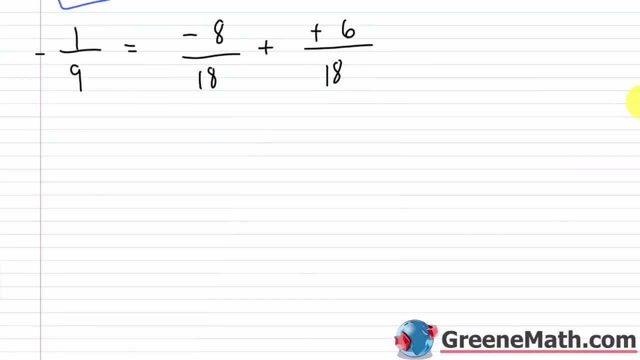 so we're good to go there now we're just checking to see if the left and the right side are equal so negative eight plus six is going to give me negative two so this would be negative two over eighteen so we get negative one ninth is equal to negative two over eighteen and this would be negative one ninth if i simplify and divide numerator and denominator by two i would have negative one over nine is equal to negative one over nine so our solution here which again was x equals negative three is correct 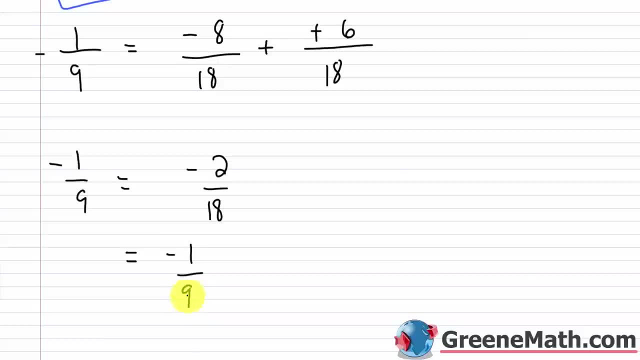 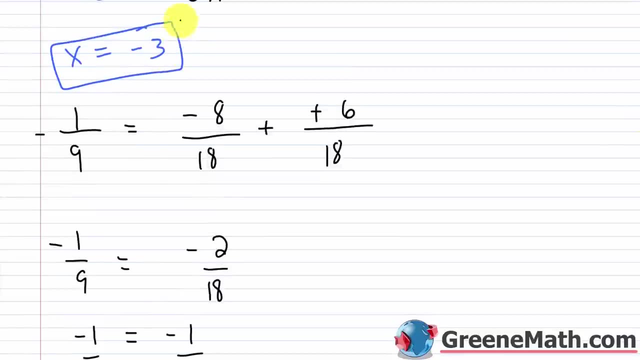 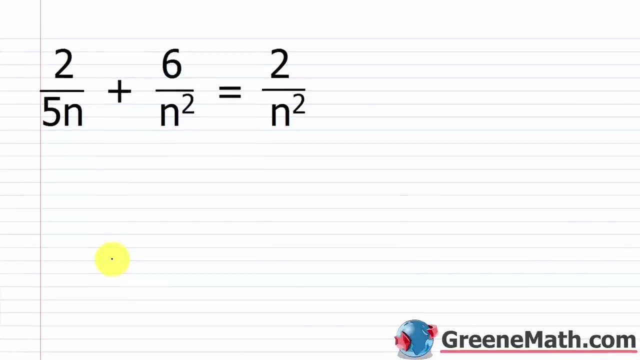 By two, I would have. negative. one over nine Is equal to negative one over nine, So our solution here, Which again was x equals negative three, Is correct. Alright, for the next one. Let's look at two over five, n Plus six over n squared. 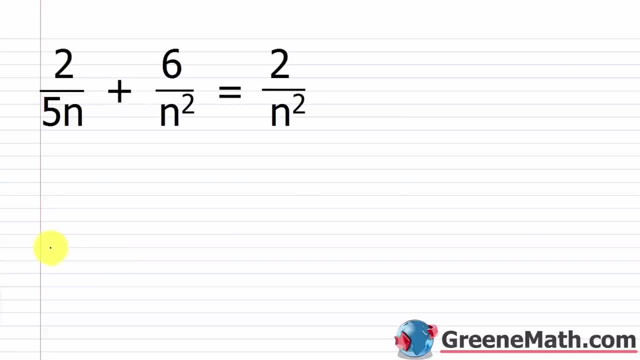 Is equal to two over n squared. So what is the LCD here? What would that be? Well, we look at the fact that I only have a number of five, No other number in any of the denominators. So that goes in there. 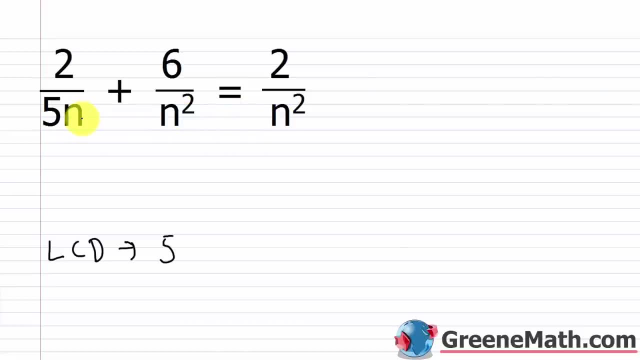 And then each has an n. This one is n squared, n squared and n. So we go with the highest exponent on the variable n, And that's a two. So we just put n squared in there. So now that that's done. 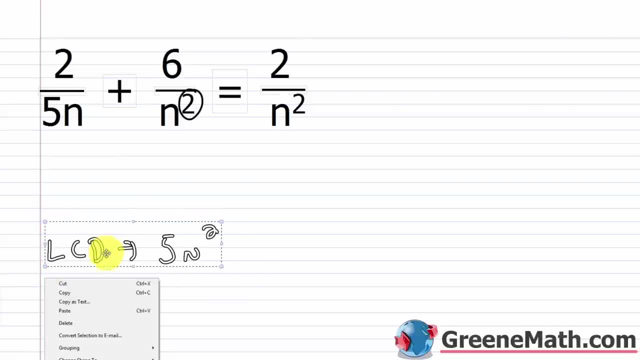 We want to multiply both sides of the equation by the LCD. So let me scooch this up, Or actually I'm going to put it up here, Make it nice and out of the way, And I would have Two over five n. 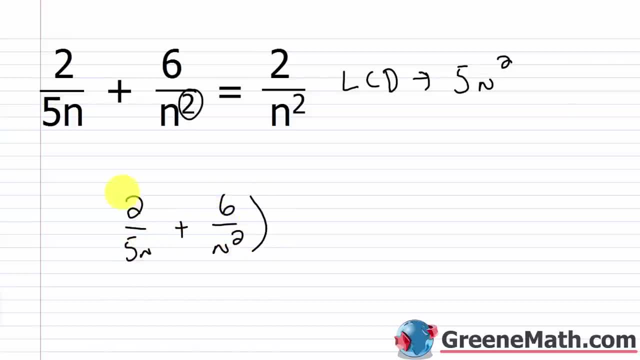 Plus six over n squared. This is going to be multiplied by five n squared, And then this is equal to Two over n squared Times five n squared. So this is going to be Now, if you wanted to take the route of seeing, 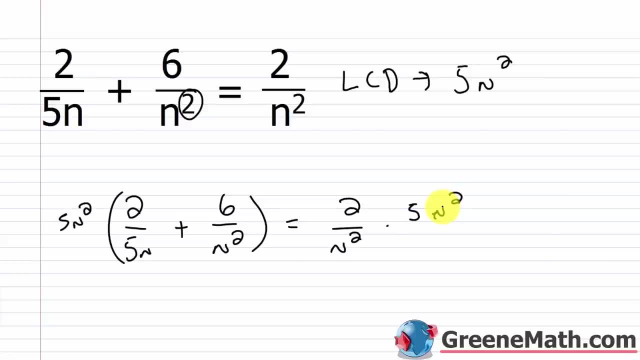 What couldn't my Variable be equal to? before I start, I could do that. I could say: okay, well, I have an n here, an n squared and an n squared. Obviously, n cannot be zero. Right, It can be anything else other than zero. 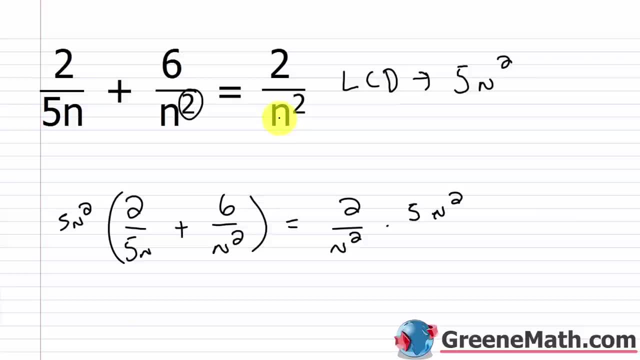 If I get a value of n equals zero, I've got to reject that solution. But just as valid- I could have not figured that out here- Figured out the problem. If I get an n net equals zero, Then I've got to reject that solution. 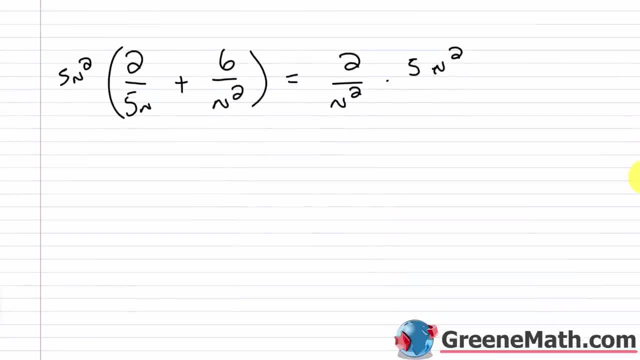 Okay, so let's go ahead And multiply. So use my distributive property: Five n squared times two over five n, The fives would cancel, And one factor of n here Would cancel with this n, And essentially I'd have n times two. 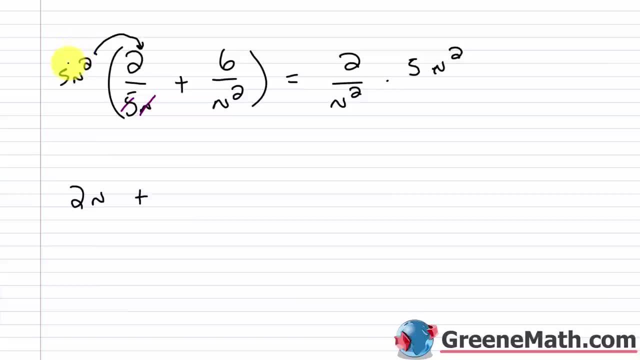 Which is just two n, Then plus Next. I would do five n squared times Six over n squared, And the n squareds are going to cancel, And essentially I'm going to have five times six, Which is thirty. Now, over here, I can just cancel this n squared. 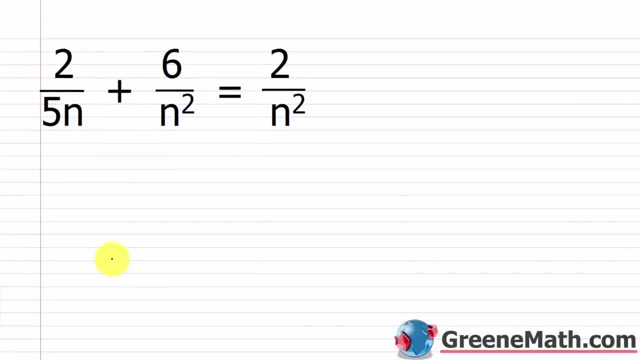 alright for the next one let's look at two over five n plus six over n squared is equal to two over n squared so what is the lcd here what would that be well we look at the fact that i only have a number of five no other number in any of the denominators so that goes in there and then each has an n this one is n squared and n so we go with the highest exponent on the variable n and that's a two right so we just put n squared in there so now that that's done 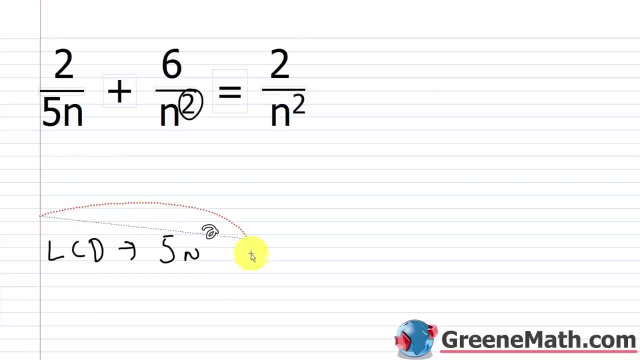 we want to multiply both sides of the equation by the lcd so let me scooch this up or actually i'm going to put it up here make it nice and out of the way and i would have two over five n plus six over n squared this is going to be multiplied by five n squared and then this is equal to two over n squared times five n squared 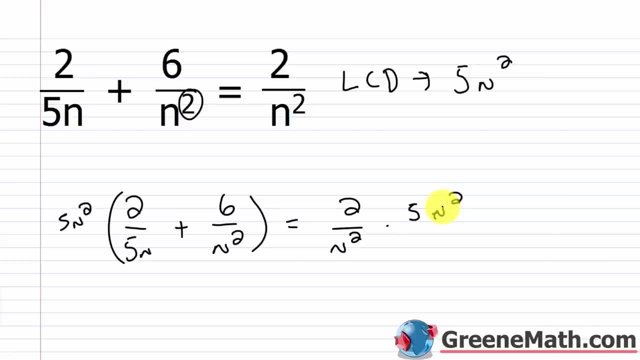 now if you wanted to take the route of seeing what couldn't my 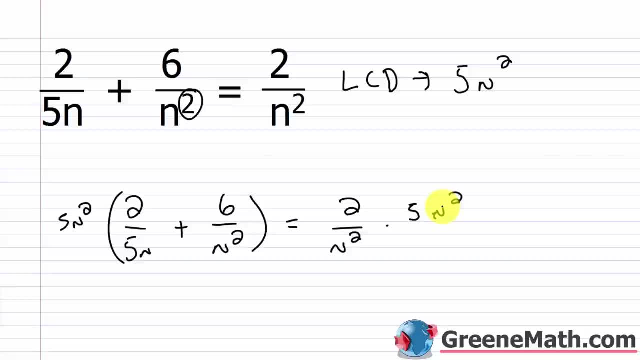 variable be equal to before i start i could do that i could say okay well i have an n here an n squared and an n squared obviously n cannot be zero right it can be anything else other than zero if i get a value of n equals zero i've got to reject that solution but just as valid i could have not figured that out here figured out the problem and then came back up and plugged it in and say okay if i get an n net equals zero then i've got to reject that solution okay so let's go ahead 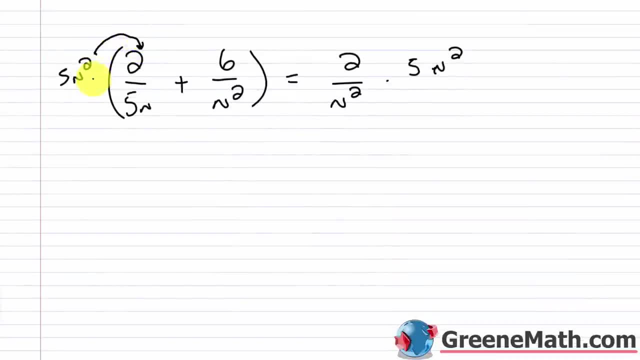 and multiply so use my distributive property five n squared times two over five n the fives would cancel and one factor of n here would cancel with this n and essentially i'd have n times two which is just two n then plus next i would do five n squared times six over n squared and the n squareds are going to cancel and essentially i'm going to have five times six which is thirty now over here i can just cancel this n squared with this n squared 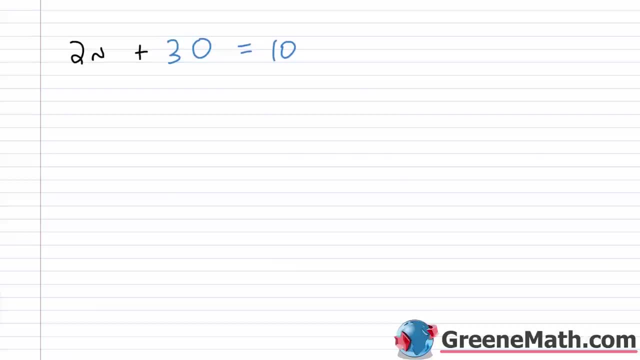 five times two is ten so this equals ten and now we have a super simple equation to solve i subtract thirty away from each side of the equation i get two n is equal to negative twenty so i divide both sides of the equation by two and i get that n is equal to negative ten 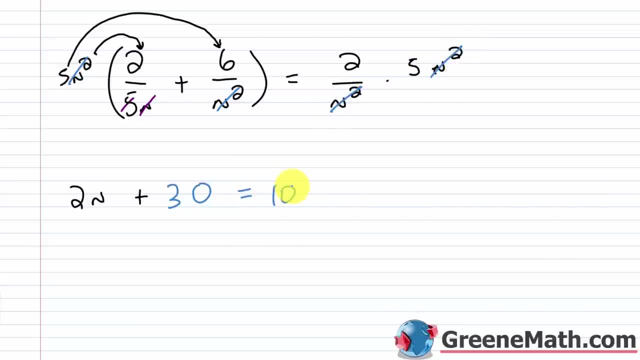 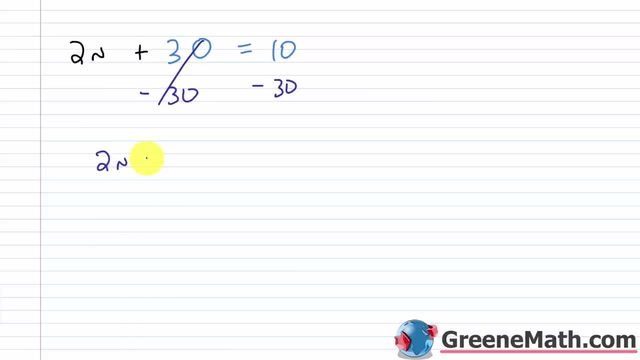 With this: n squared Five times two is ten, So this equals ten. And now we have a super simple equation to solve. I subtract thirty away from each side of the equation, I get two. n is equal to Negative twenty. So I divide both sides of the equation by two. 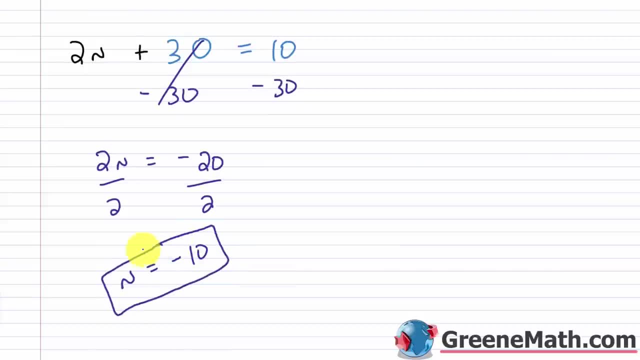 And I get that n is equal to negative ten. Okay, So that is not zero. So I know we don't have to reject the solution, But we still want to check it to make sure That we got the right answer- So important that we do that when we start out. 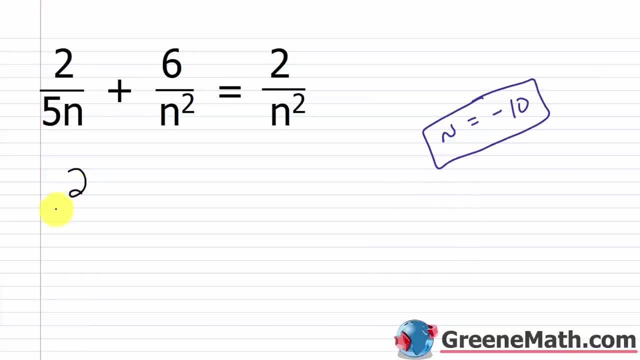 Okay, so again, n is equal to negative ten. So I'm looking at two over Five times negative ten. Just plug in a negative ten for n Plus six over. If I square negative ten, I get a hundred. This equals two over. 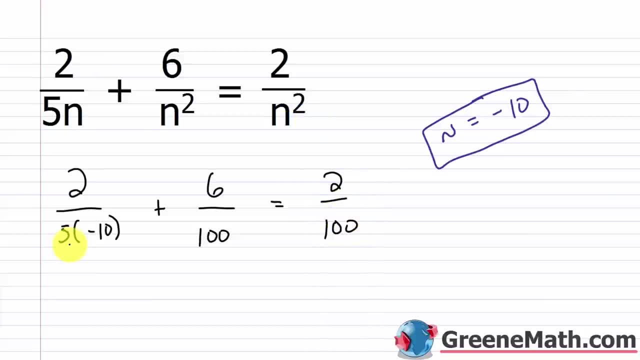 Again, if I square negative ten, I get a hundred. So over here, If I multiply five times negative ten, I would have negative fifty. Now I need to get a common denominator going. So I'm going to do two things. I'm going to move this negative up into the numerator. 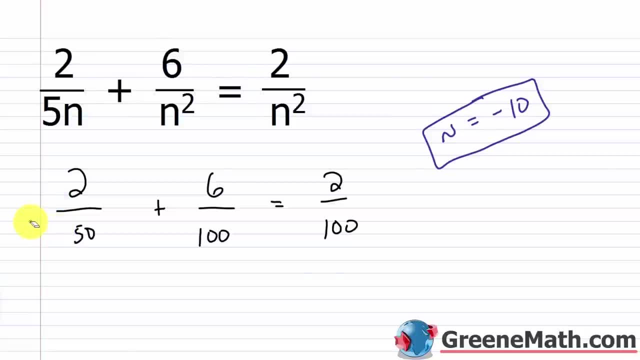 Remember that's perfectly legal. And then I'm going to Multiply both Numerator and denominator by two, And so this is going to be negative four over one hundred. Negative four over one hundred. Negative four over one hundred. So negative four plus six is two. 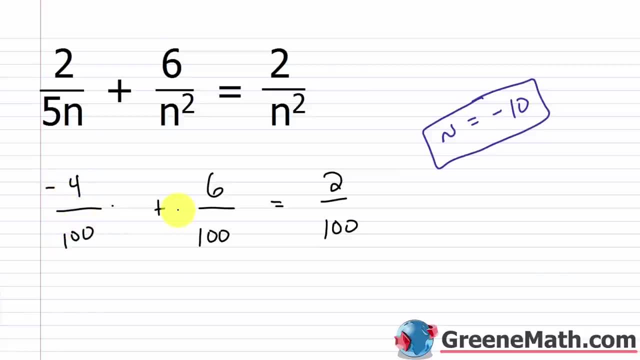 So this side would be two over a hundred, And this side is two over a hundred, And this side is two over a hundred And this side is two over a hundred. You could simplify each side to one over fifty if you wanted to. 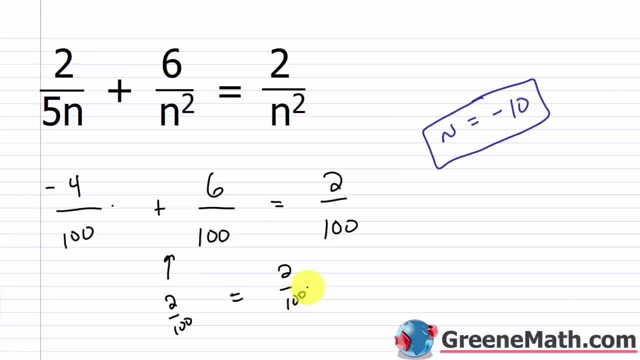 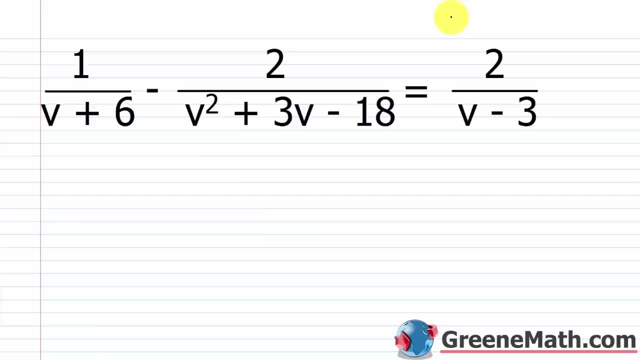 But you're just trying to see That the left and the right side are equal, Which they are. So again you can say that your solution here N equals negative ten is correct. Alright, for the next one, I'm looking at One over V plus six. 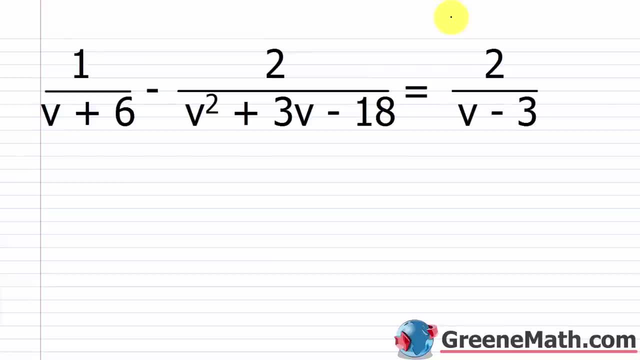 Minus two over V. squared Plus three, V minus eighteen, This is equal to two over V minus three. Alright, So this one is going to be a little bit more time consuming, But still not very hard overall. But still not very hard overall. 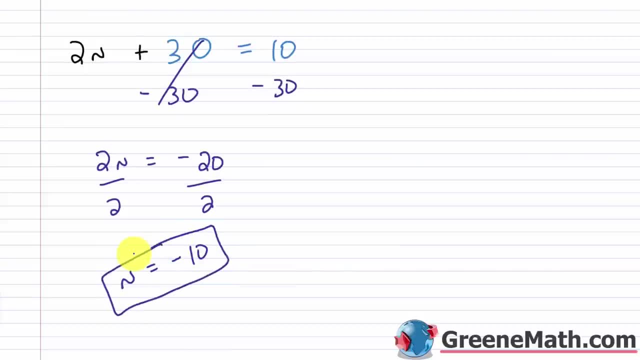 okay so that is not zero so i know we don't have to reject the solution but we still want to check it to make sure that we got the right answer so important that we do that when we start out okay so again 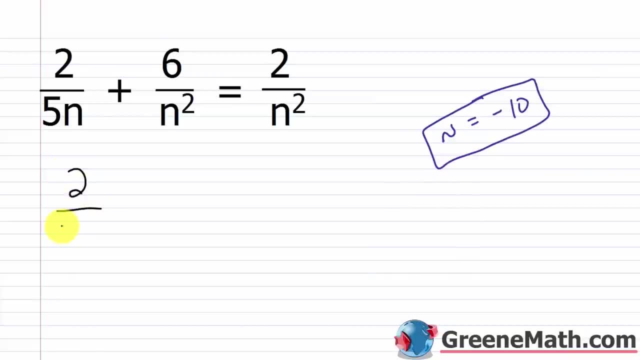 n is equal to negative ten so i'm looking at two over five times negative ten just plug in a negative ten for n plus six over if i square negative ten i get a hundred this equals two over again if i square negative ten i get a hundred so over here if i multiply five times negative ten i would have negative fifty now i need to get a common denominator going so i'm going to do two things i'm going to move this negative up into the numerator remember that's perfectly legal 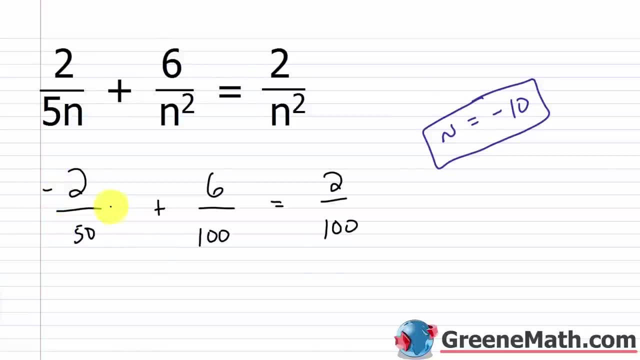 and then i'm going to multiply both numerator and denominator by two and so this is going to be negative four over one hundred negative four over one hundred so negative four plus six is two so this side would be two over a hundred and this side is two over a hundred you could simplify each side to one over fifty if you wanted to but you're just trying to see that the left and the right side are equal which they are so again you can say that your solution 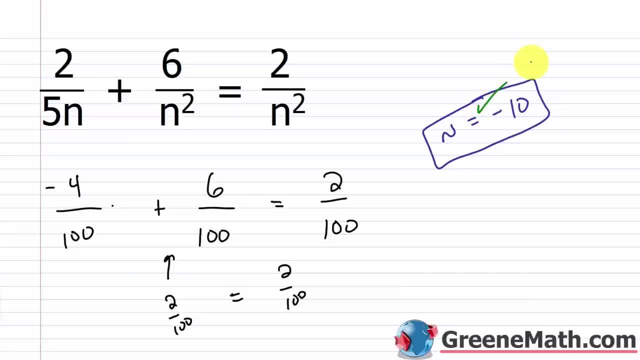 here n equals negative ten is correct 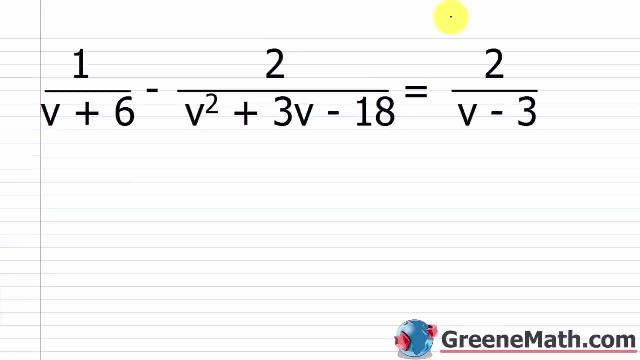 alright for the next one i'm looking at one over v plus six minus two over v squared plus three v minus eighteen this is equal to two over v minus three 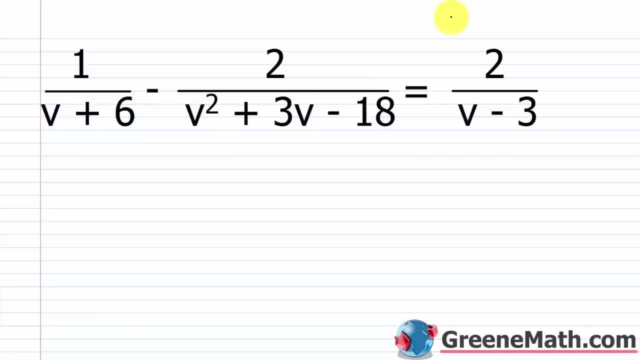 alright so this one's going to be a little bit more time consuming but still not very hard overall the lcd here is the first thing we want to find so the lcd what is that well for this denominator i have v plus six for this one 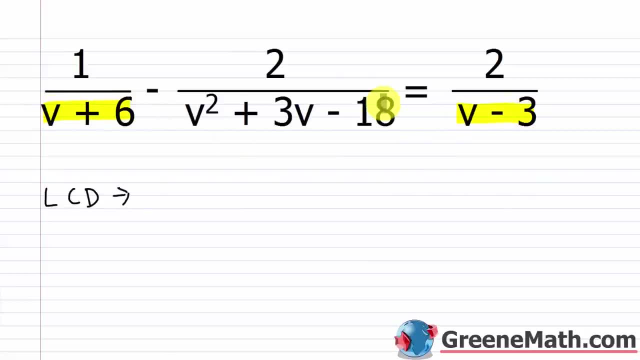 i have v minus three it's pretty straight forward for this one i need to factor it to see what's going on now when you first start getting these problems particularly in algebra one you're going to be able to guess that one of these at least is going to be a factor of this in this particular case it's going to factor perfectly to give you those two so give me two integers so you're going to have v plus six and v minus three so you'd have v plus six 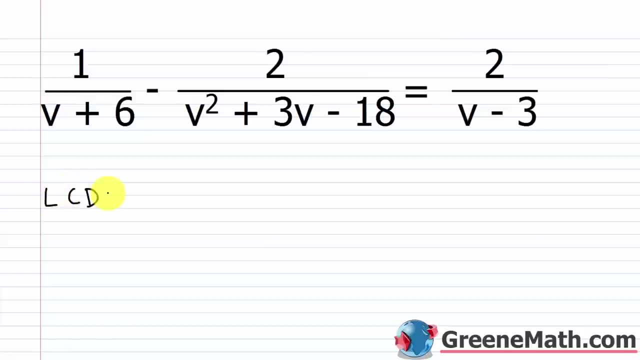 The LCD. here is the first thing we want to find. So the LCD. What is that? Well, for this denominator, I have V plus six. For this one, I have V minus three. It's pretty straight forward For this one. I need to factor it to see what's going on. 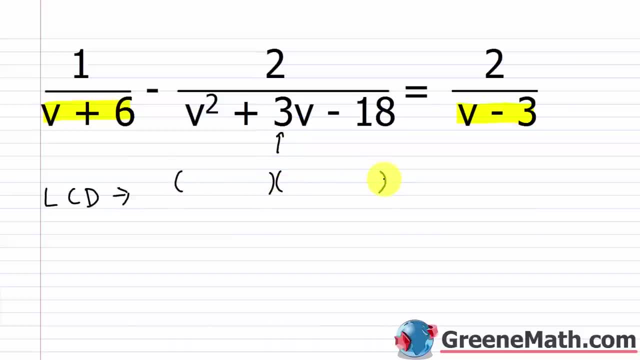 Now, when you first start getting these problems, Particularly in algebra one, You're going to be able to guess That one of these at least, Is going to be a factor of this. In this particular case, You need to factor perfectly to give you those two. 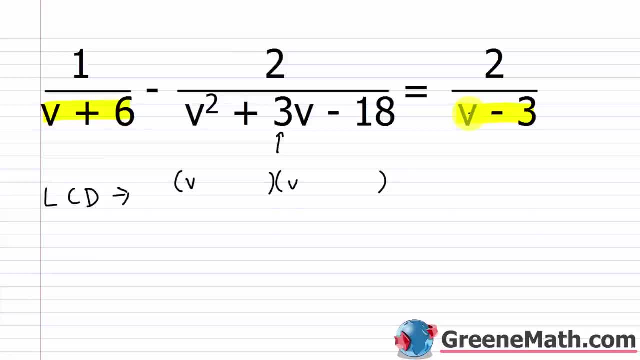 So give me two integers Whose sum is three And whose product is negative eighteen. Well, of course, that's going to be positive six And negative three, So you'd have V plus six and V minus three. So your LCD is just that. 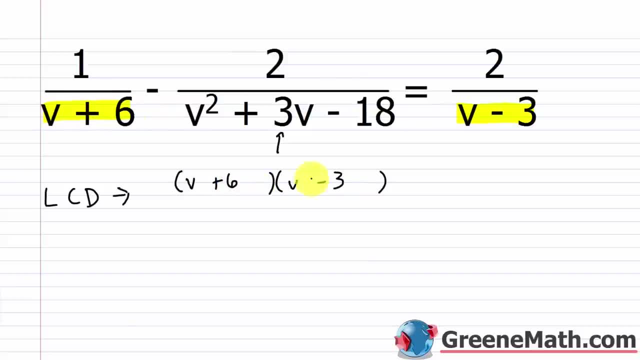 It's V plus six, Which occurs here and here, And V minus three, which occurs here and here. So once you have that, The V plus six Times V minus three, You want to multiply it by eight By each side of the equation. 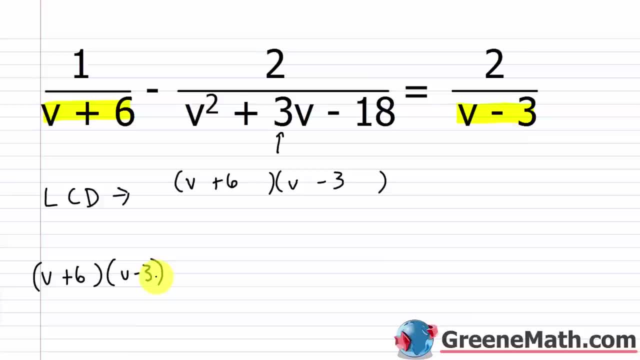 Because of the length of my screen, I don't think I could possibly Fit all of this in there. So, without having to scroll back and forth What I'm going to do, I'm just going to say that I'm going to be multiplying this. 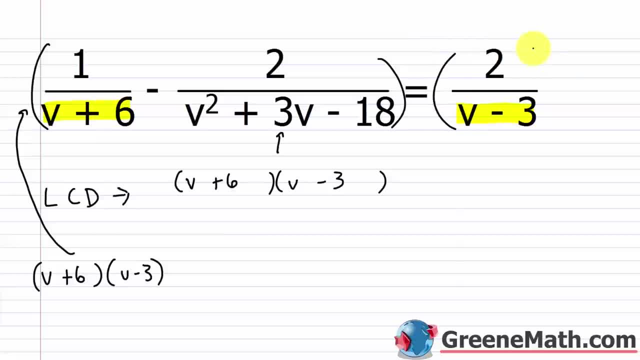 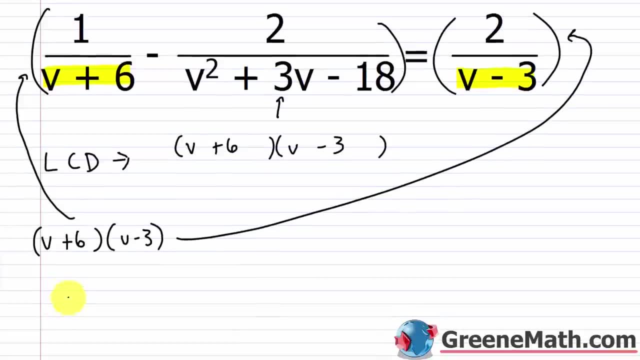 By this side of the equation. So I'm going to multiply by this side And I'm also going to multiply it by that side. But I'm just going to do the work down here And then just report the simplified result. So if I had V plus six, 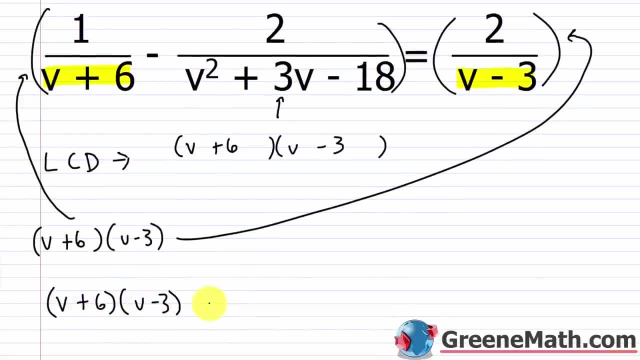 Times V minus three, And I multiply this by One over V plus six. Obviously the V plus six Would cancel here and here And I'd just be left with V minus three. So for the first one Let me kind of scroll down. 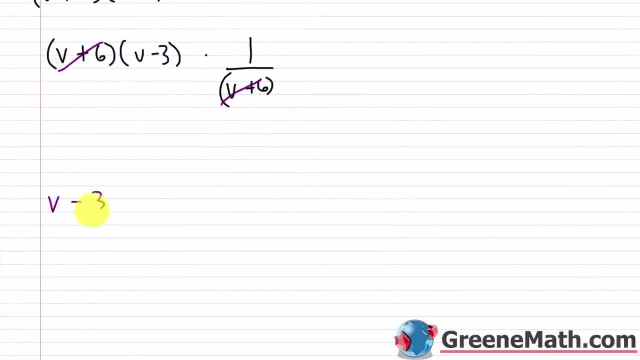 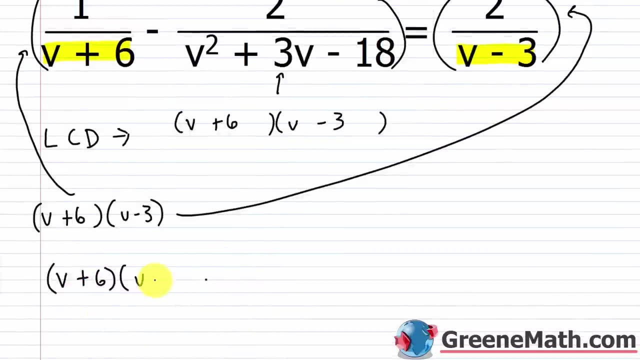 I would have just a V minus three. Okay, Let me scroll back up now And I'll just be going back and forth. So this was V minus three here. So now I'm going to multiply by this guy here. Now the denominator here. 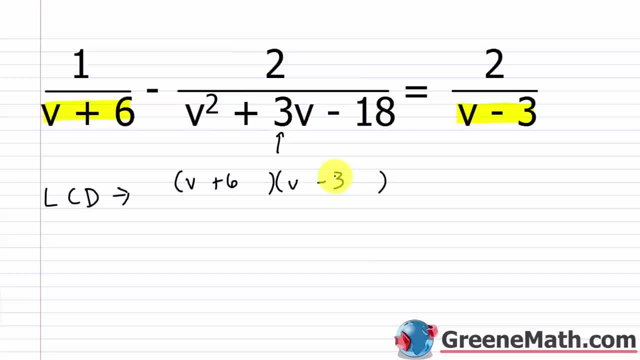 and v minus three so your lcd is just that it's v plus six which occurs here and here and v minus three 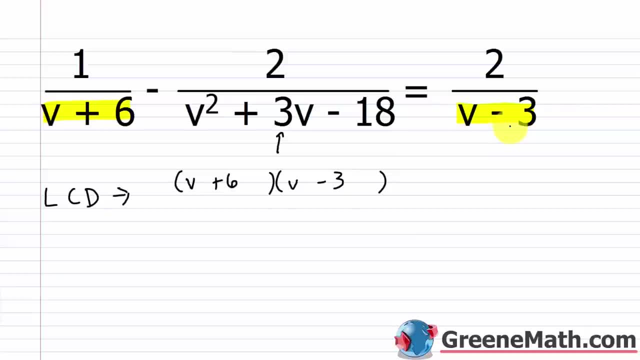 which occurs here and here so once you have that the v plus six times v minus three 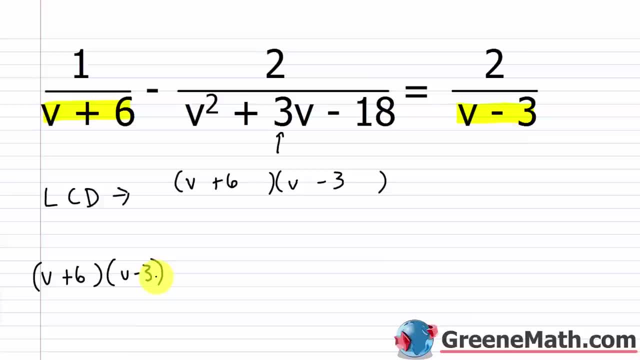 you want to multiply it by each side of the equation because of the length of my screen i don't think i could possibly fit all of this in there so without having to scroll back and forth what i'm going to do i'm just going to say that i'm going to be multiplying 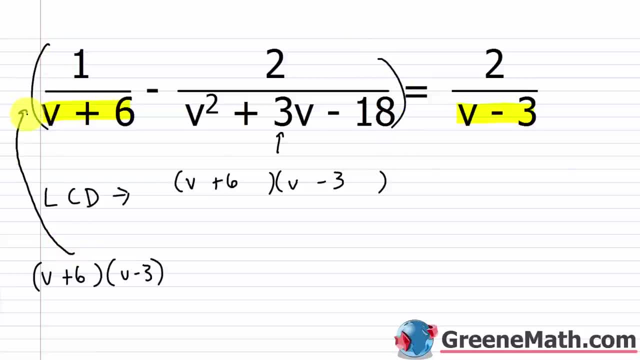 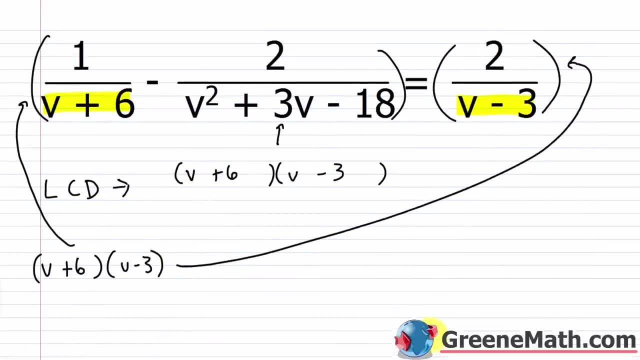 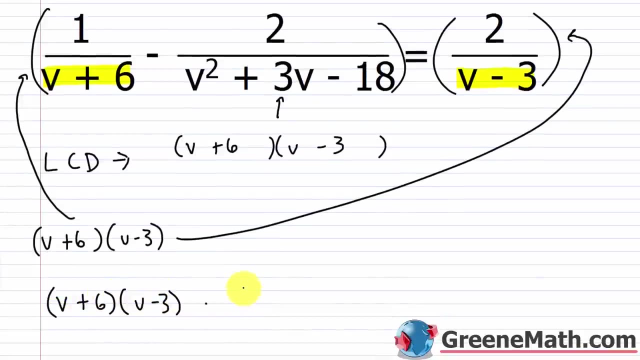 this by this side of the equation so i'm going to multiply by this side and i'm also going to multiply it by that side but i'm just going to do the work down here and then just report the simplified result so if i had v plus six times v minus three and i multiply this by one over v plus six obviously the v plus six would cancel here and here and i'd just be left with v minus three so for the first one let me kind of scroll down i would have just a v minus three 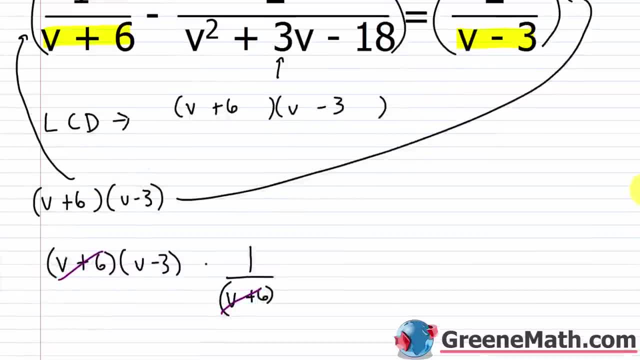 ok let me scroll back up now and i'll just be going back and forth so this was v minus three here 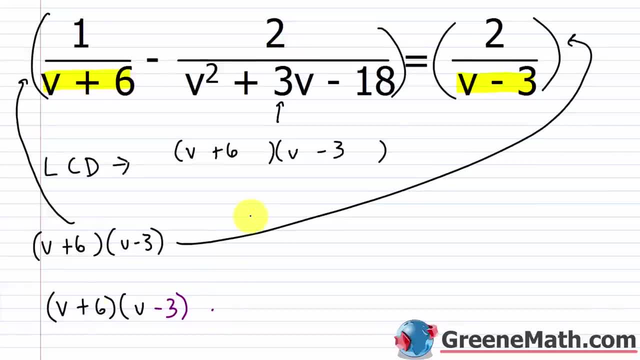 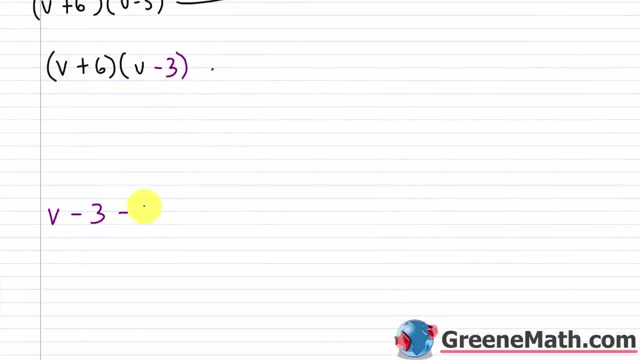 so now i'm going to multiply by this guy here now the denominator here is exactly this so we know that without even going through this the denominator here is going to cancel with this right here and i'm just going to be left with a minus two so if i was to write this over here i would simply put minus two now 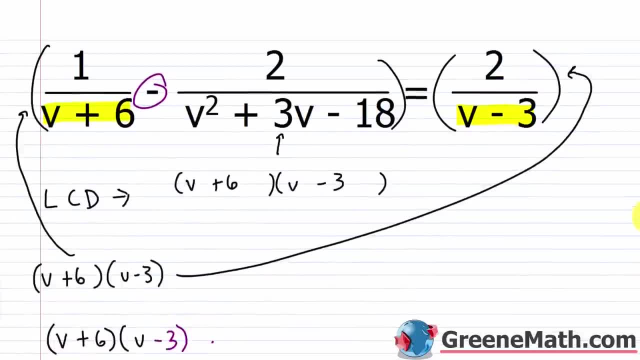 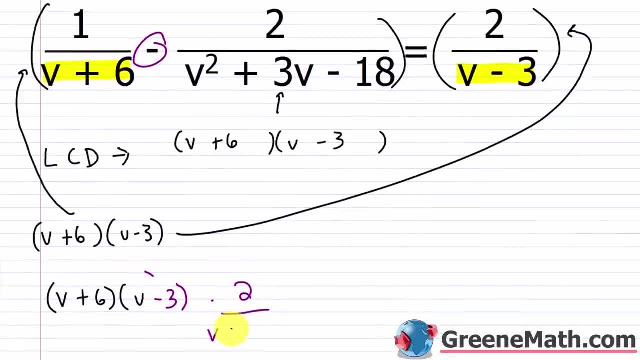 then equals i would be on this side now and i would be multiplying this guy right here by two over v minus three so v minus three cancels with v minus three and i've got two times the quantity v plus six so two times the quantity v plus six 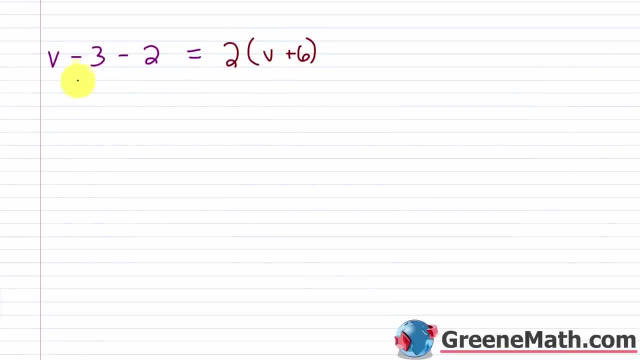 ok so let's simplify each side and go ahead and solve so negative three minus two is minus five so v minus five is equal to two times v is two v 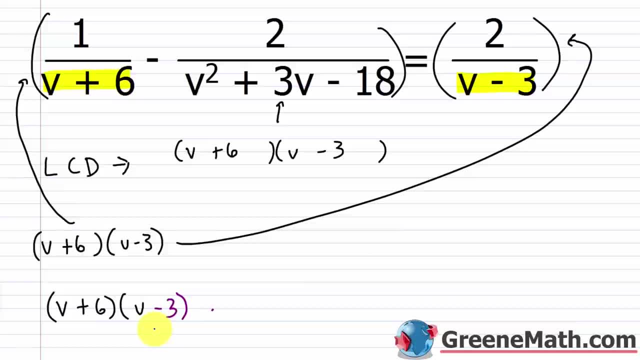 Is exactly this. So we know that, without even going through this, The denominator here Is going to cancel with this right here, And I'm just going to be left with a minus two Right. So if I was to write this over here, 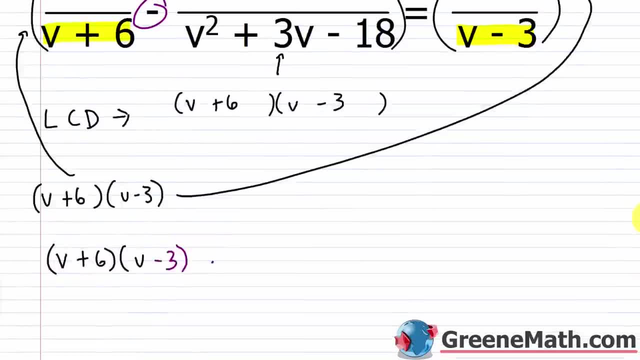 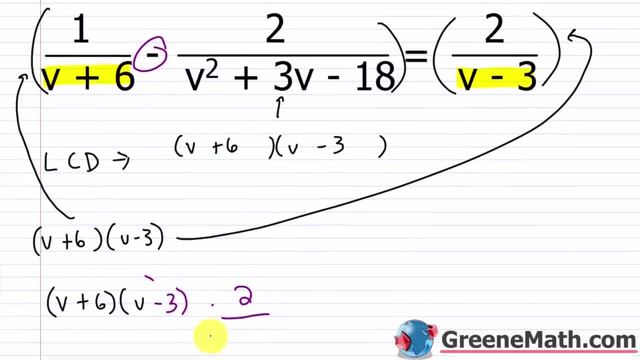 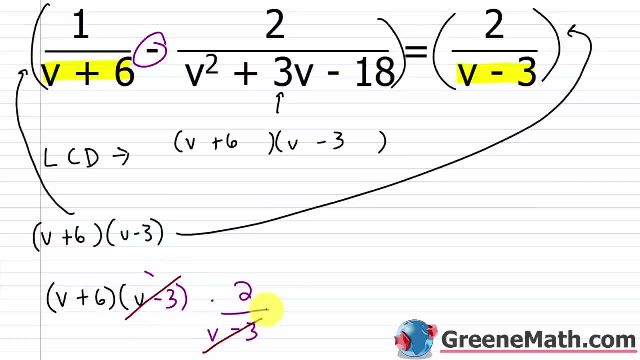 I would simply put minus two now, Then equals. I would be on this side now And I would be multiplying This guy right here By two over V minus three. So V minus three Cancels with V minus three And I've got two times the quantity V plus six. 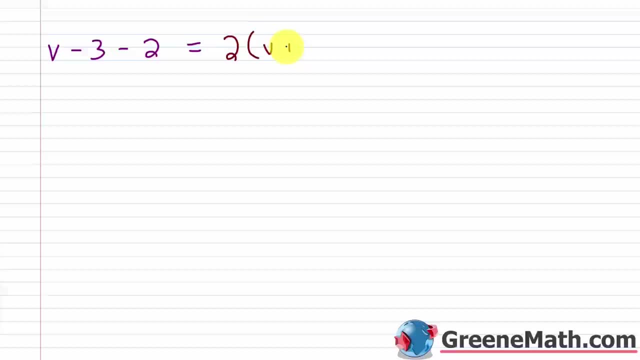 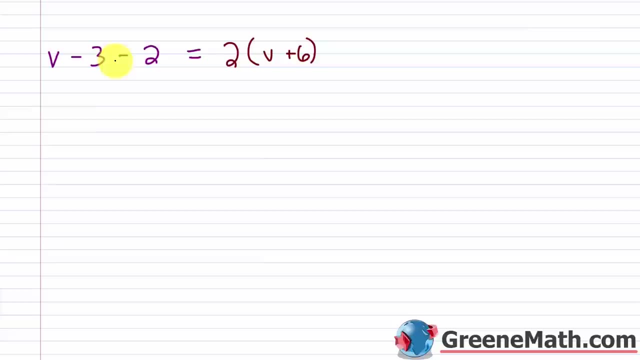 So two times the quantity V plus six. Okay, So let's simplify each side And go ahead and solve So negative. three minus two is minus five. So V minus five Is equal to: two times V is two V, And then two times six is twelve. 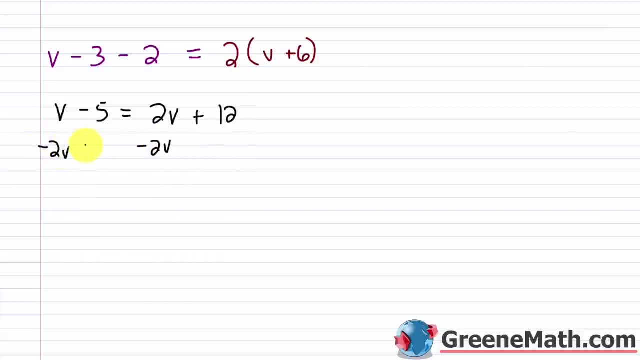 If I subtract two V away From each side of the equation And add five to both sides of the equation, What is that going to give me? This is going to cancel And this is going to cancel. On the left side. I'm going to have negative V. 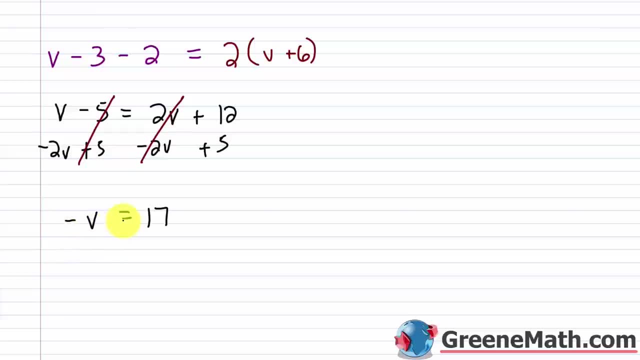 On the right side, I'm going to have seventeen. So the opposite of V is seventeen. That means V is negative seventeen. Right, I can show that by multiplying both sides by negative one, Or dividing both sides by negative one. Whatever you want to do. 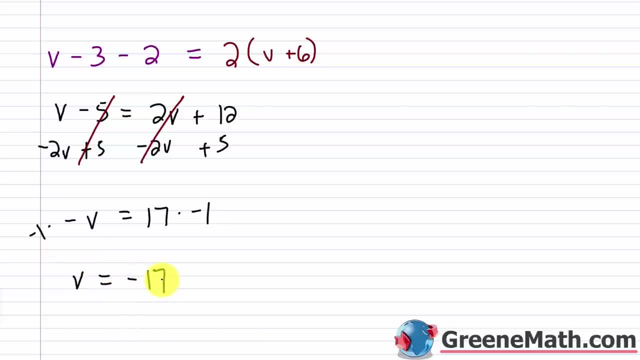 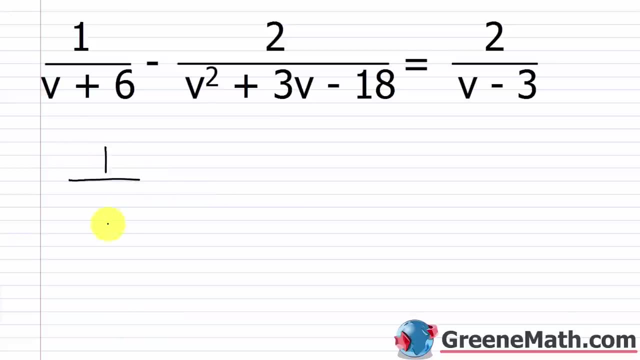 That gives me V is equal to negative seventeen. Okay, Let's erase everything And then we're going to go back and check. This is going to be easier for me. So one over, You'd have negative seventeen plus six Minus two over. 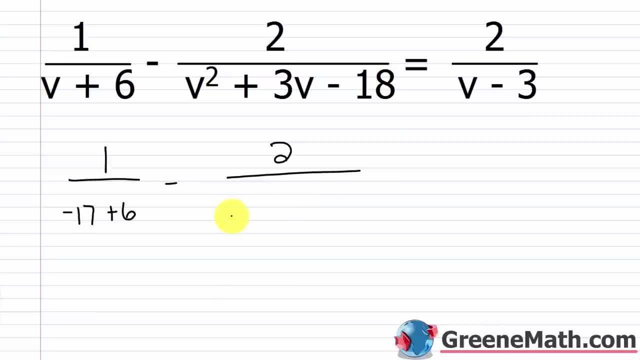 You have again V plus six, So that's negative seventeen plus six, And that's multiplied by V minus three, So negative seventeen minus three. These two quantities are multiplied together. This is multiplication, So make sure you don't just write it as one long string. 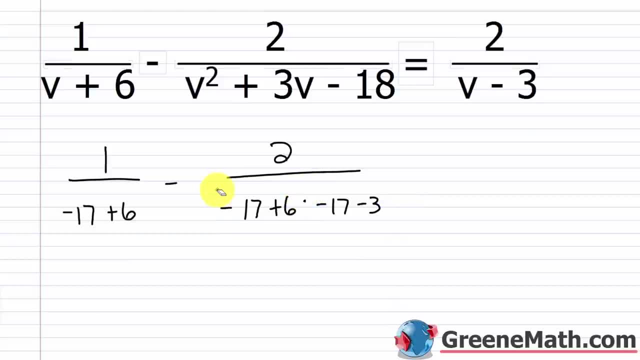 Because it's easy to just kind of Substitute it in that way, Realize that it's multiplication And make a mistake. So it's: this times this, Then this equals two over. You've got negative seventeen minus three. So let's crank this out real quick. 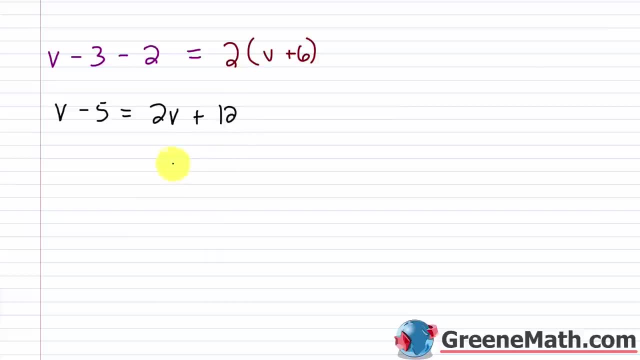 and then two times six is twelve if i subtract two v away from each side of the equation and add five to both sides of the equation what is that going to give me this is going to cancel and this is going to cancel on the left side i'm going to have negative v on the right side i'm going to have seventeen so the opposite of v is seventeen that means v is negative seventeen i can show that by multiplying both sides by negative one or dividing both sides by negative one whatever you want to do 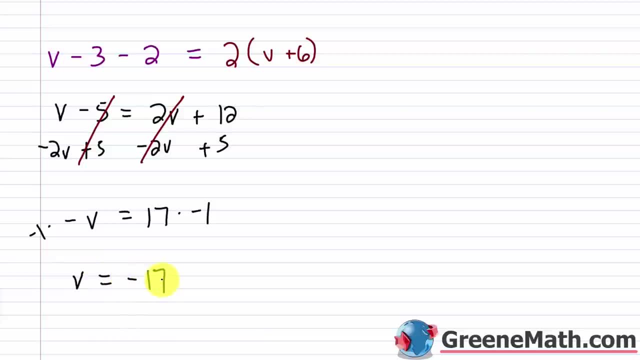 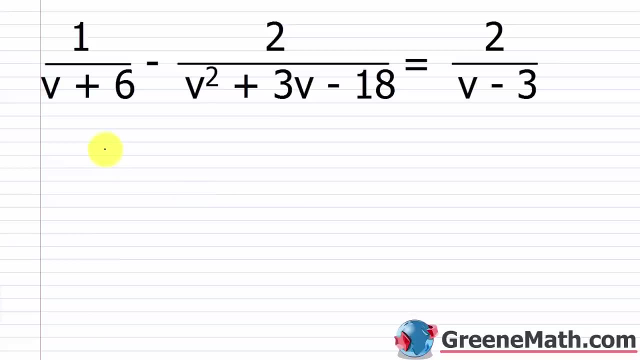 that gives me v is equal to negative seventeen ok let's erase everything and then we're going to go back and check and i'm going to use the factor denominator to check it's just going to be easier for me so one over you'd have negative seventeen plus six minus two over you have again v plus six so that's negative seventeen plus six and that's multiplied by v minus three so negative seventeen minus three these two 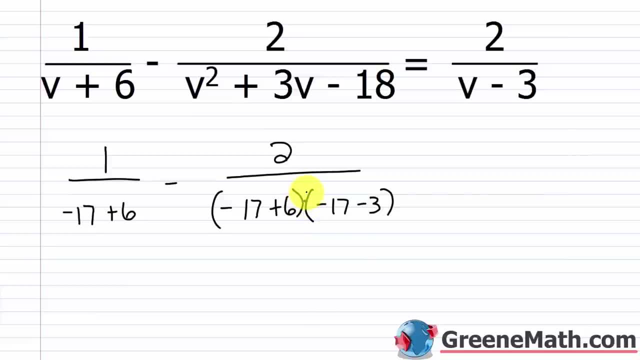 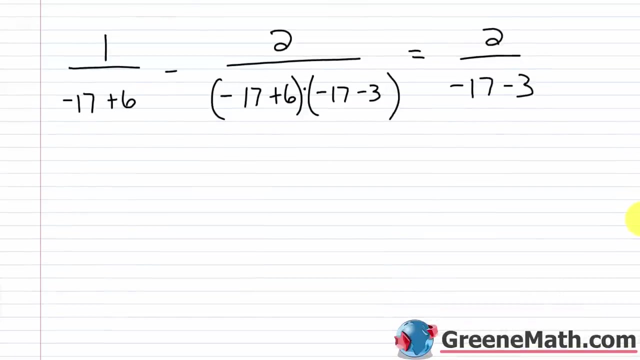 quantities are multiplied together this is multiplication so make sure you don't just write it as one long string because it's easy to just kind of substitute it in that way and not realize that it's multiplication and make a mistake so it's this times this then this equals two over you've got negative seventeen minus three so let's crank this out real quick negative seventeen plus six is negative eleven so i've got one over negative eleven or i can write negative one over eleven does not 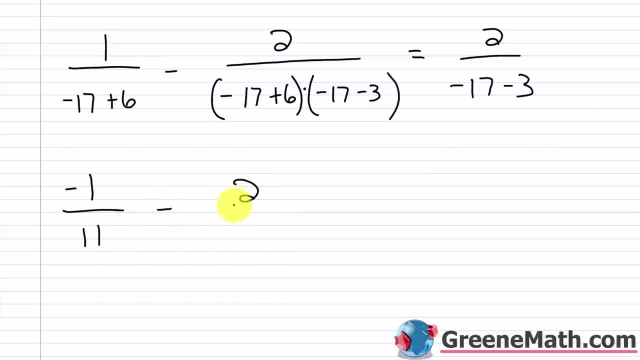 matter and then we're subtracting away we have two over negative seventeen plus six is negative eleven negative seventeen minus three is negative twenty so if i multiply these two together i know i'm going to get a positive so what is two times eleven well that's twenty two then just put your zero at the end the trailing zero that gives you two hundred twenty 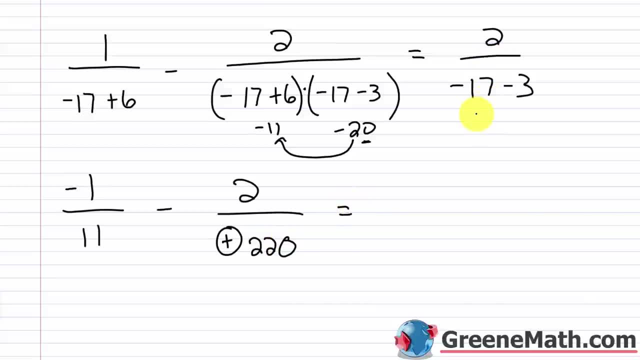 now this is going to be equal to two over negative seventeen minus three so that's two over negative twenty 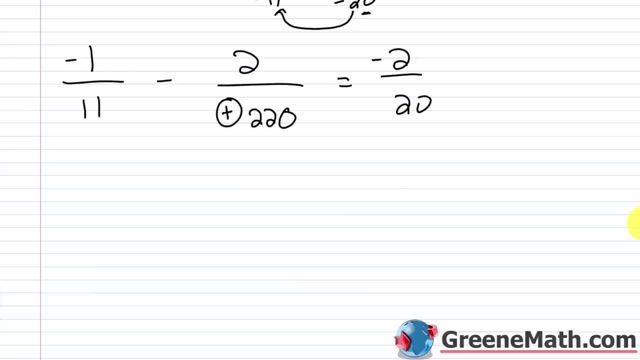 or again i could write this as negative two over twenty doesn't matter so now what i want to do just go through and simplify as 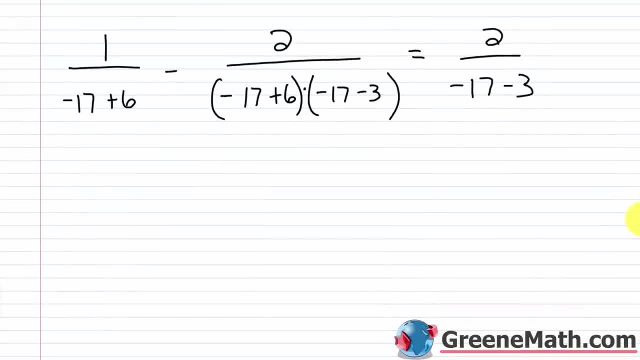 Negative. seventeen plus six Is negative eleven. So I've got one over negative eleven. Or I can write negative one over eleven, Does not matter, And then we're subtracting away. We have two over Negative. seventeen plus six is negative eleven. 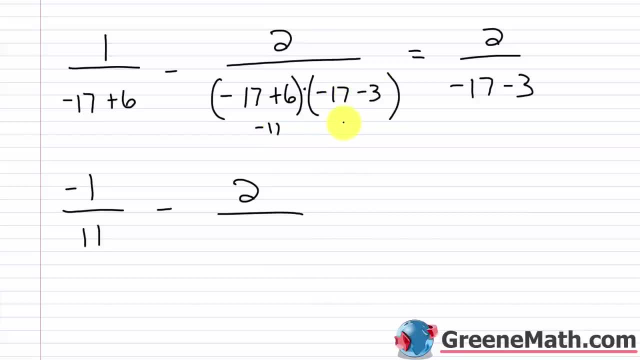 Negative seventeen minus three Is negative twenty. So if I multiply these two together, I know I'm going to get a positive. So what is two times eleven? Well, that's twenty two. Then just put your zero at the end, The trailing zero. 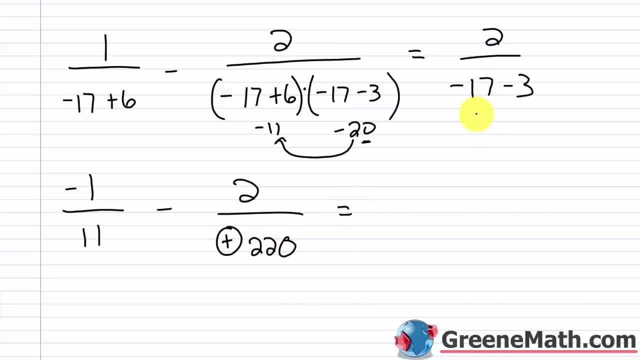 That gives you two hundred twenty. Now this is going to be equal to Two over negative seventeen minus three. So that's two over negative twenty. Or again I could write this as Negative two over twenty. Doesn't matter, I'm just going to simplify as much as I can. 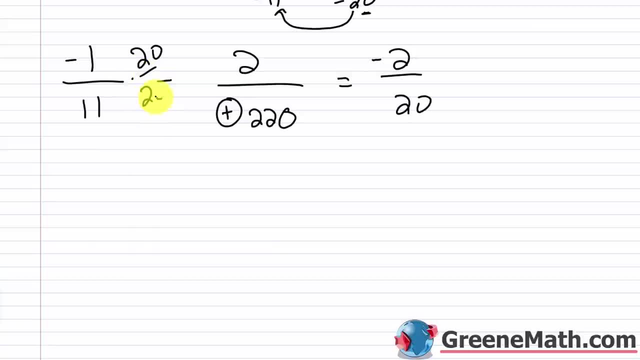 So I need to multiply this By twenty over twenty So I can have a common denominator. So twenty times negative one is negative twenty. So I'd have negative twenty minus two Over a common denominator of two hundred twenty. So this would be negative twenty two. 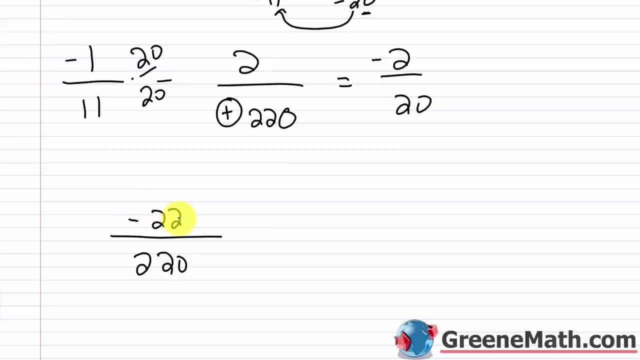 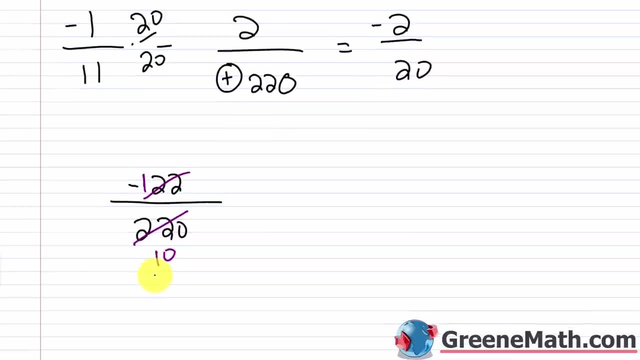 Over two hundred twenty. And what would that reduce to? Well, each is divisible By twenty two. Twenty two divided by twenty two is one, So this would be negative one. And two hundred twenty Divided by twenty two is ten, So this is negative one. tenth, 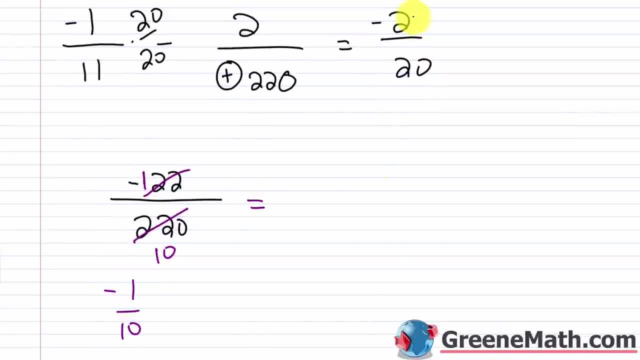 So let me write that right there. This is equal to: If I divide this by two, I get one. If I divide this by two, I get ten. So again, negative one, tenth. And let me write it down here for the sake of completeness. 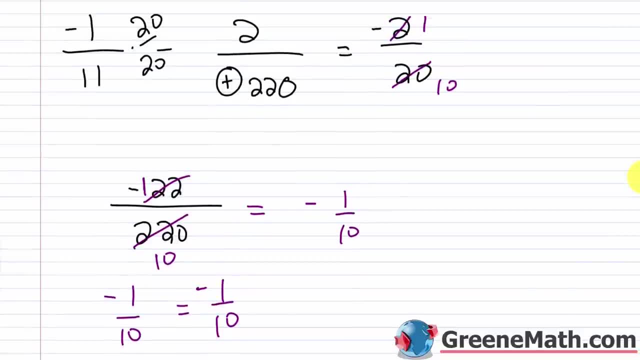 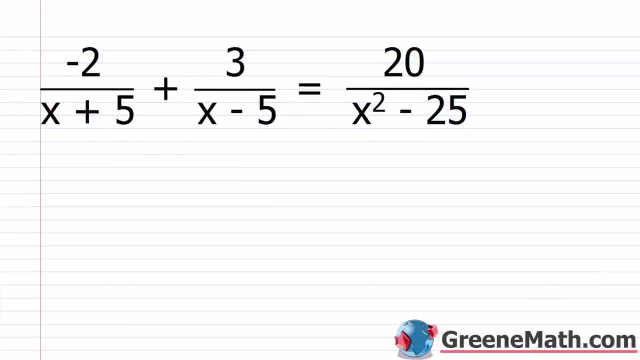 We get: negative one tenth Is equal to negative one tenth. So our solution, Which we have down here: V equals negative seventeen is correct. Alright, for the next one, We're going to take a look at Plus three over x minus five. 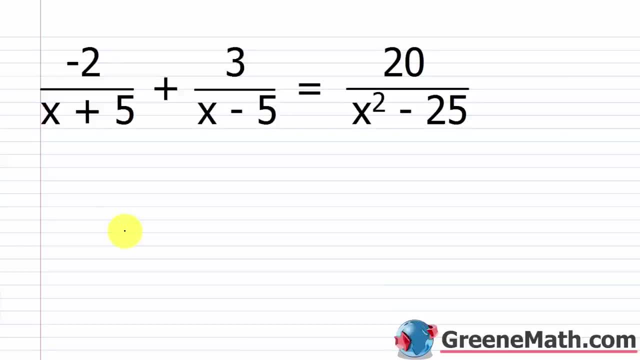 Is equal to Twenty over x squared minus twenty five. So for the LCD, You can see here that X squared minus twenty five is what It's the difference of two squares. It's x plus five Times x minus five, And this matches what you have here and here. 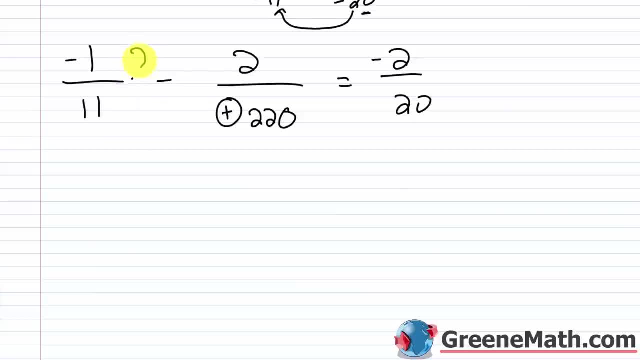 much as i can so i need to multiply this by twenty over twenty so i can have a common denominator so twenty times negative one is negative twenty so i'd have negative twenty minus two over a common denominator of two hundred twenty 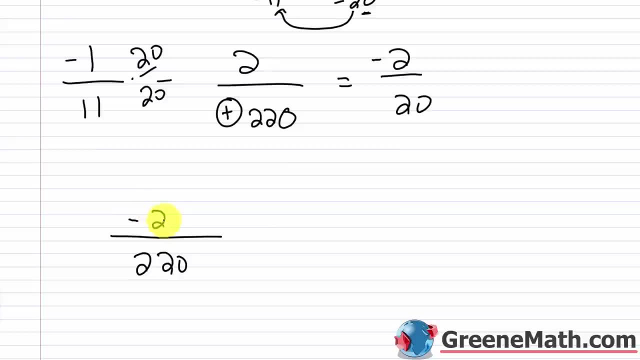 so this would be negative twenty two over two hundred twenty and what would that reduce to well each is divisible by 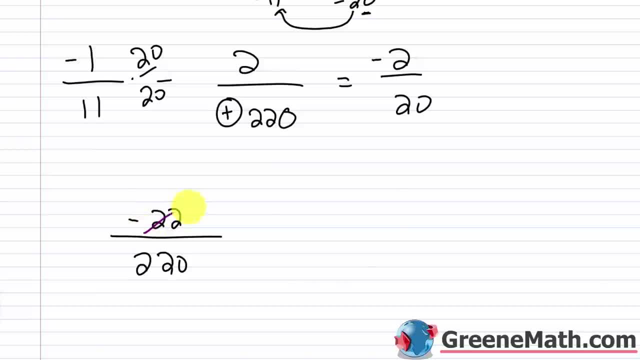 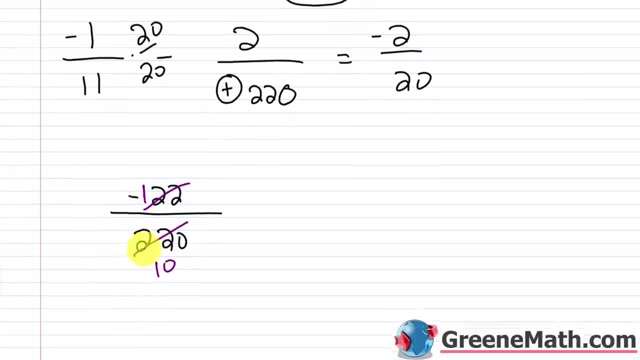 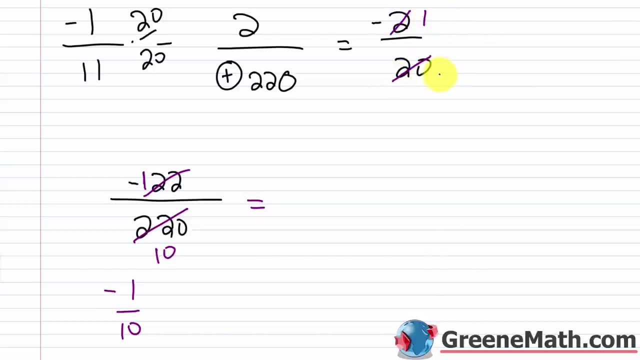 twenty two twenty two divided by twenty two is one so this would be negative one and two hundred twenty divided by twenty two is ten so this is negative one tenth so let me write that right there this is equal to if i divide this by two i get one if i divide this by two i get ten so again negative one tenth and let me write it down here for the sake of completeness we get negative one tenth is equal to negative one tenth so our solution which we have down here v equals negative seventeen is correct 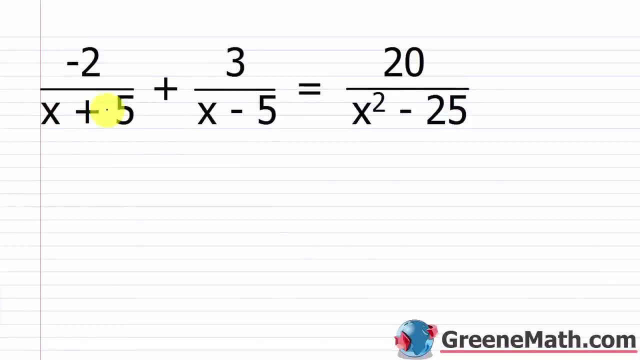 alright for the next one we're going to take a look at negative two over x plus five plus three over x minus five is equal to twenty over x squared minus twenty five so for the lcd you can see here that x squared minus twenty five is what it's the difference of two squares it's x plus five times x minus five and this matches what you have here and here 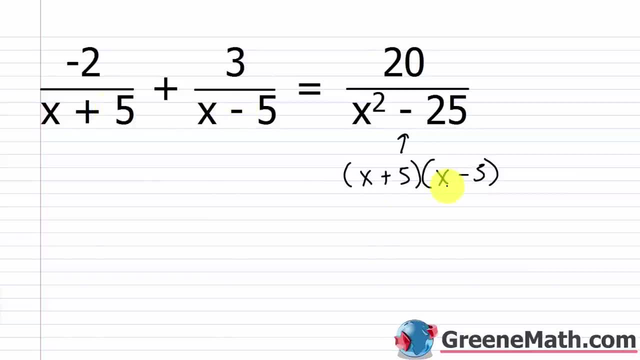 so the lcd is just this the quantity x plus five times the quantity x minus 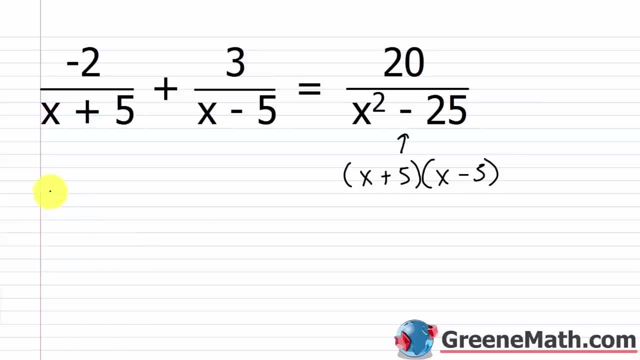 five so if i multiplied let me just write that the lcd is that if i multiplied both sides of the equation by this what would happen if i multiply this part right here by the lcd the x plus five would cancel with the x plus five here right so what i'd have is a negative two a negative two times the quantity x minus five then plus in this particular case when i multiply this lcd by this the x minus five is 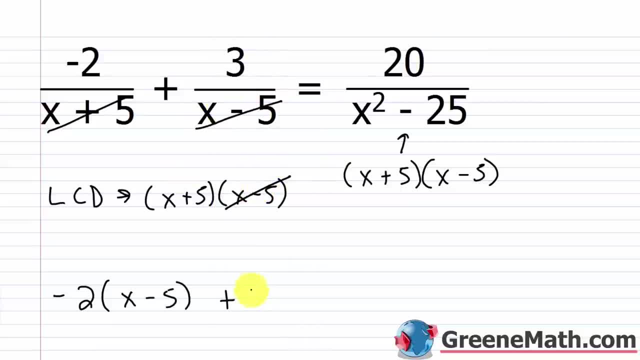 going to cancel and it'll cancel here so i'd have three times the quantity x plus five 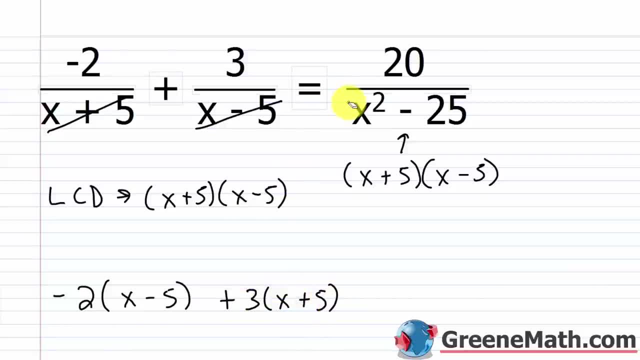 in this particular case once i get past the equal sign over here i have x plus five times x minus five so this is going to cancel completely with this right this denominator would just cancel 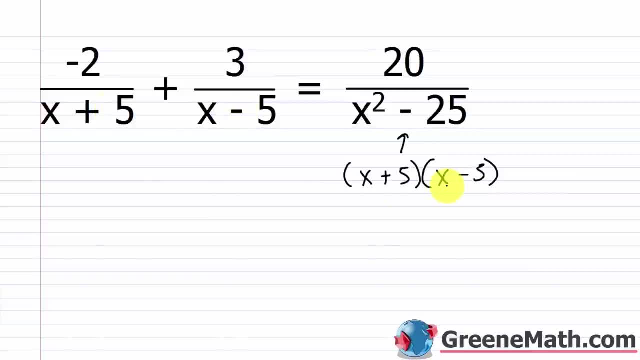 So the LCD is just this: The quantity x plus five times the quantity x minus five. So if I multiplied, Let me just write that- the LCD is that If I multiplied Both sides of the equation by this, What would happen If I multiply this part right here? 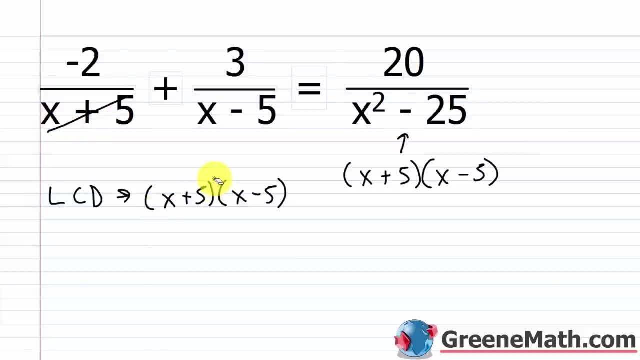 By the LCD. The x plus five would cancel with the x plus five here. So what I'd have is a negative two, A negative two Times the quantity x minus five, Then plus In this particular case, when I multiply this LCD. 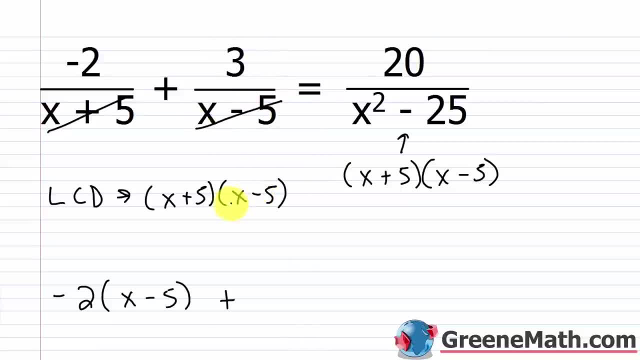 By this The x minus five is going to cancel, And it would cancel here With the quantity x plus five In this particular case. Once I get Past the equal sign over here, I have x plus five times x minus five. 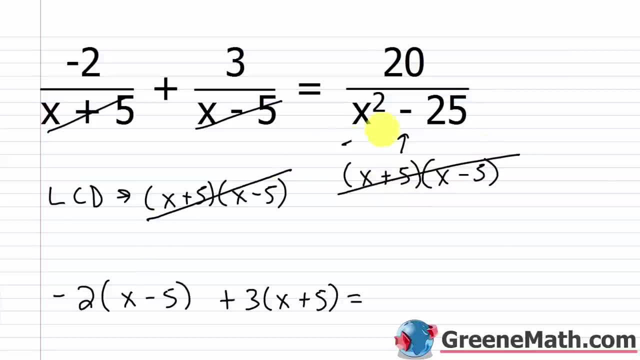 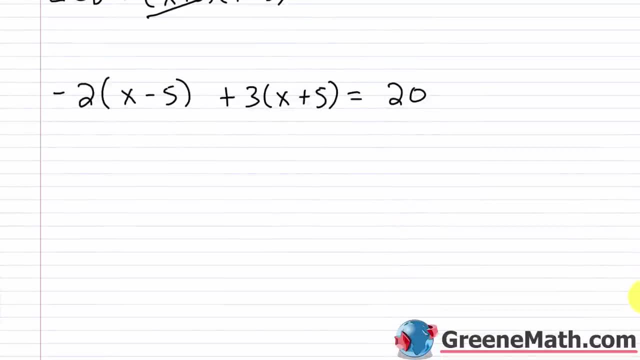 So this is going to cancel Completely. with this, This denominator would just cancel itself out And I'll simply just have twenty. So now to solve this guy: Negative two times x is negative two x. Negative two times negative five is plus ten. 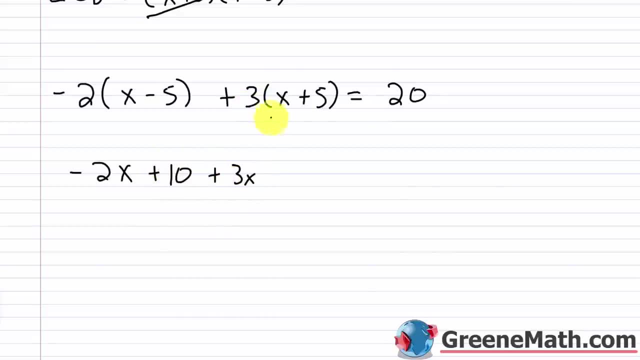 Three times x is plus three x. Three times five is plus ten. Three times five is fifteen, And this equals twenty. Now to simplify Negative: two x plus three x is x. Ten plus fifteen is twenty five, And this equals twenty. 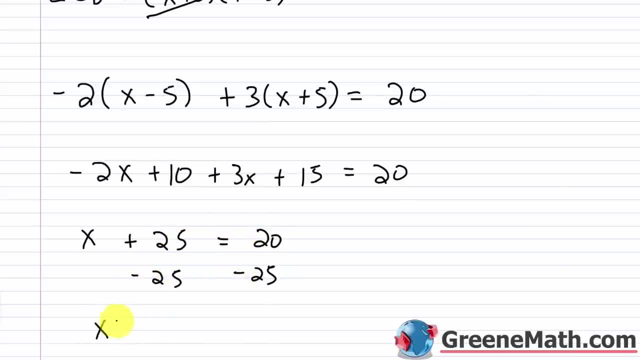 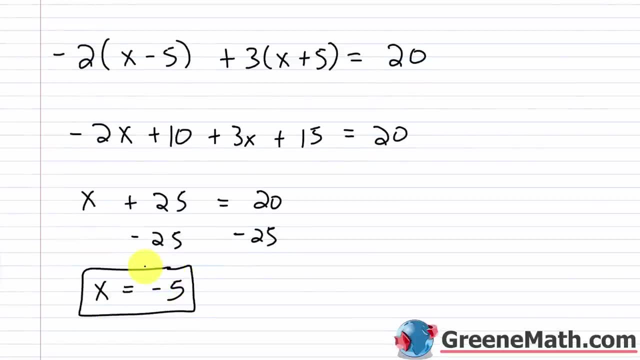 Subtract twenty five away from each side of the equation And I get that x is equal to negative five. So some of you will already see a problem, But let's go back up and substitute it in Before we say anything. Let's go back up here. 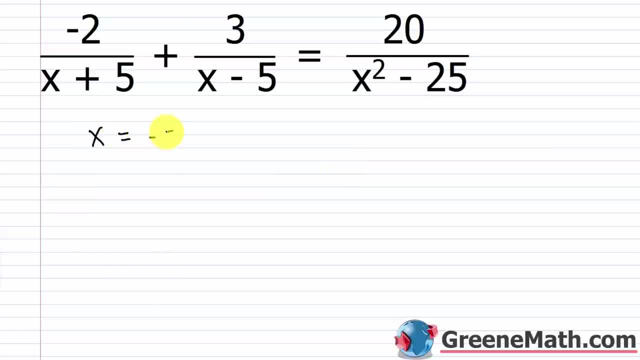 Let's erase. If x is equal to negative five, What's going to happen here When I plug a negative five in for x here And here I'm going to have a problem If I plug in a negative five for x there. 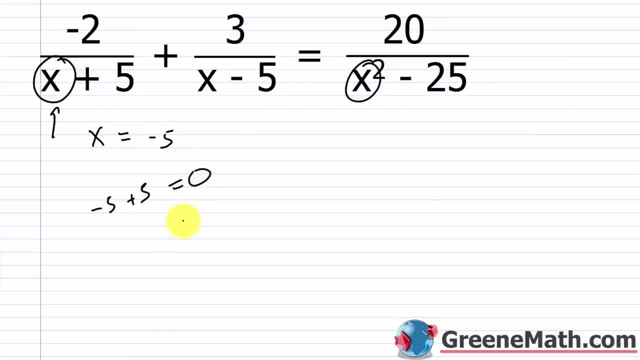 I would have negative five plus five. That equals zero. Division by zero is not allowed And if we get a result like that, We have to reject the solution. We reject: x equals negative five. It is not a valid solution If I plugged it in here. 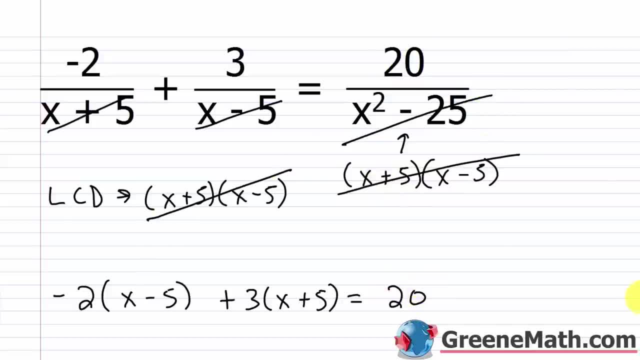 itself out and i'll simply just have twenty so now to solve this guy negative two times x is negative two x negative two times negative five is plus ten 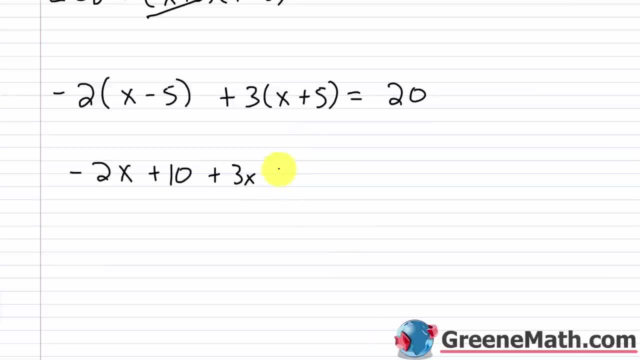 three times x is plus three x three times five is fifteen and this equals twenty 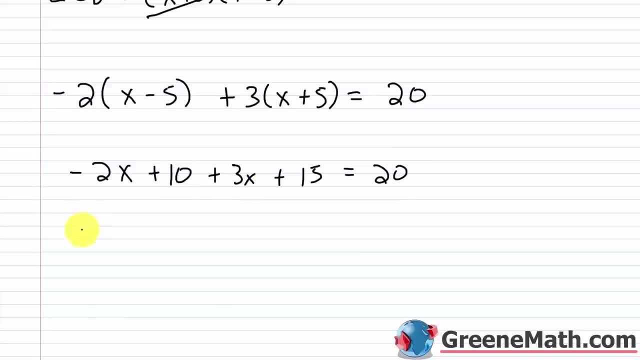 now to simplify negative two x plus three x is x ten plus fifteen is twenty five 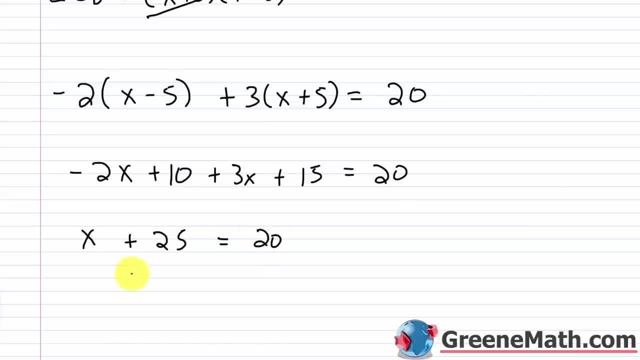 and this equals twenty subtract twenty five away from each side of the equation 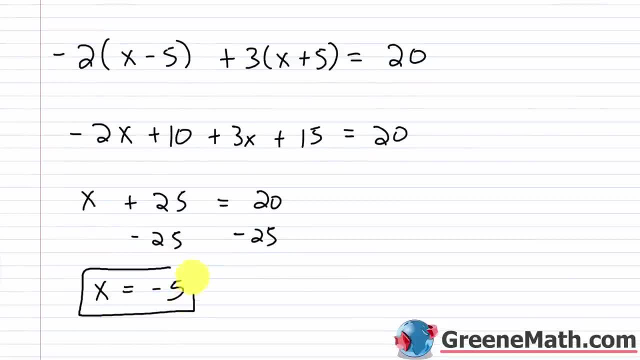 and i get that x is equal to negative five 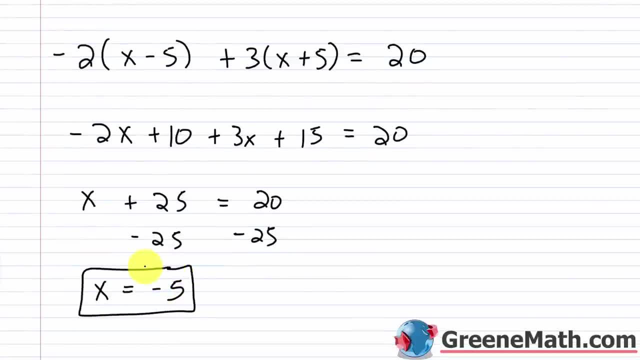 so some of you will already see a problem but let's go back up and substitute it in before we say anything let's go back up here let's erase 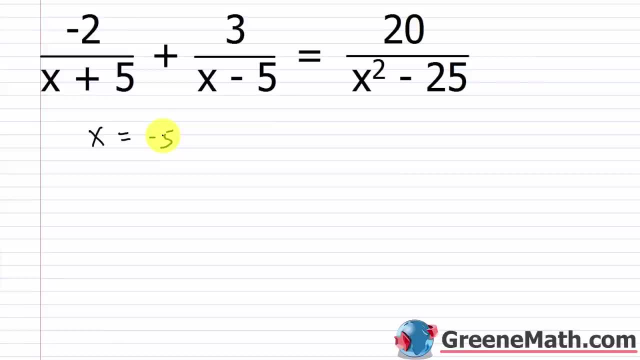 if x is equal to negative five what's going to happen here when i plug a negative five in for x here and here i'm going to have a problem right if i plug in a negative five for x there i would have negative five plus five that equals zero division by zero is not allowed and if we get a result like that we have to reject the solution we reject x equals negative five it is not a valid solution 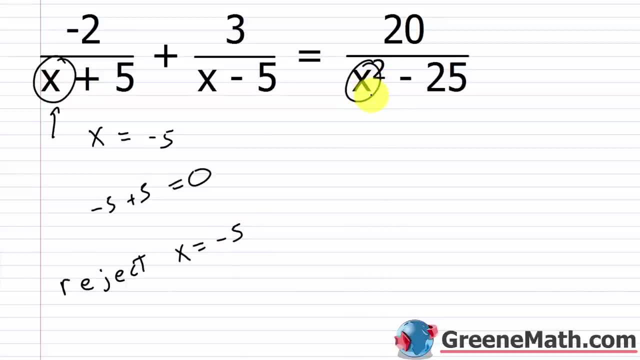 if i plugged it in here negative five that quantity squared would be twenty five twenty five minus twenty five is zero can't have that you could plug it in here negative five minus five is negative ten but that doesn't matter if it fails in one of the denominators you have to reject it you can never divide by zero so that's what you're looking for here you reject x equals negative five let me just put a big you know x through it and say it's not a solution and so we don't have a solution here we just say that there's no solution there's no solution alright 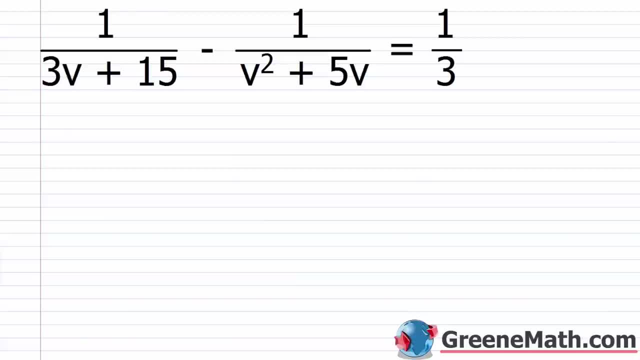 let's take a look at one more problem and we're going to wrap this up 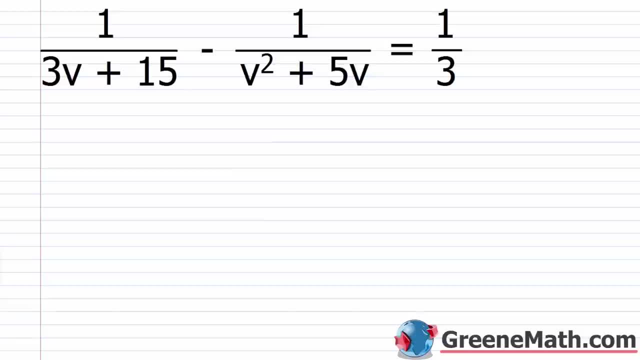 again very very easy to do this you just find the LCD multiply both sides of your equation by the LCD and then you just solve the equation like you normally would the only thing is you can't have division by zero so you've got to check that result so you don't get something like we did in the last problem 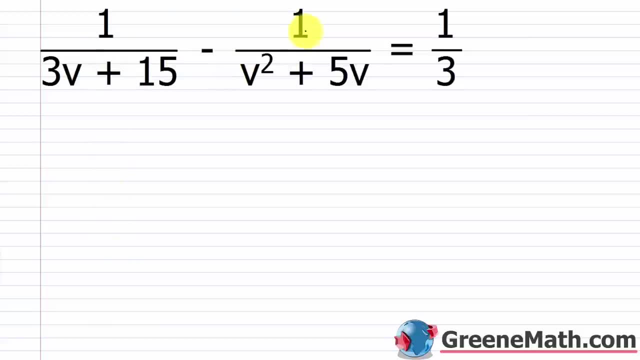 so to start this one over three v plus fifteen minus one over v squared plus five v 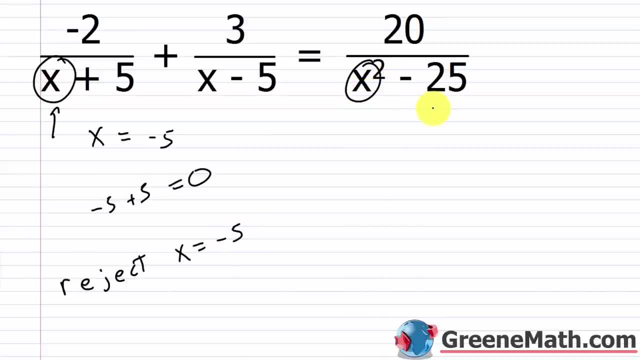 Negative five, That quantity squared Would be twenty five. Twenty five minus twenty five is zero. Can't have that. You could plug it in here. Negative five minus five is negative ten. But that doesn't matter If it fails in one of the denominators. 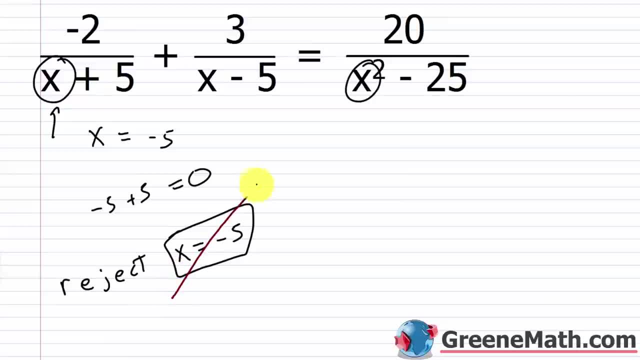 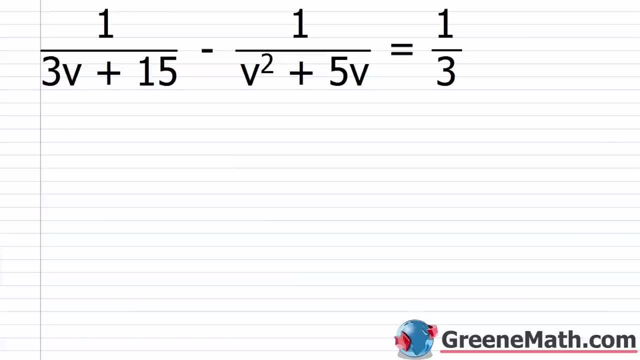 You have to reject it. You can never divide by zero, So that's what you're looking for here. You reject x equals negative five. Let me just put a big. There's no solution. There's no solution. Alright, Let's take a look at one more problem. 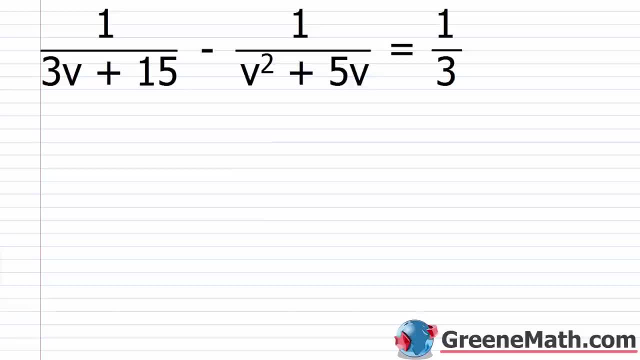 Then we're going to wrap this up Again. Very, very easy to do this. You just find the LCD, Multiply both sides of your equation by the LCD And then you just solve the equation like you normally would. The only thing is: 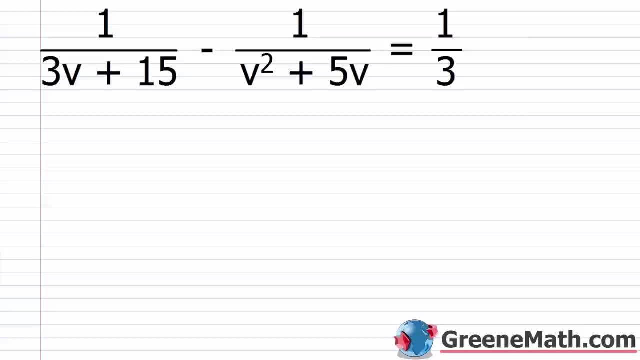 You can't have division by zero, So you've got to check that result So you don't get something like we did in the last problem. So to start this, One over three v plus fifteen Is equal to one third, So again, 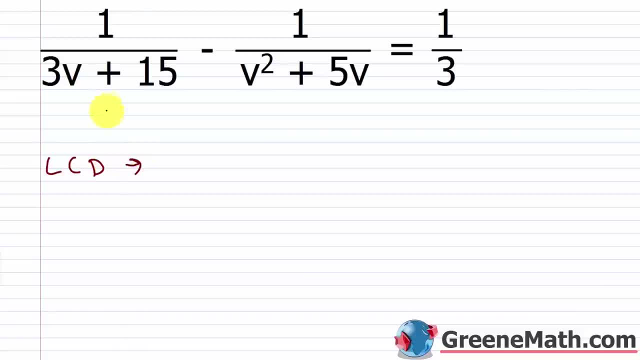 I'm looking for the LCD And for this guy I've got to factor it. It can factor into three times the quantity v plus five. For this guy I can factor out a v And I have v plus five. And for this guy, 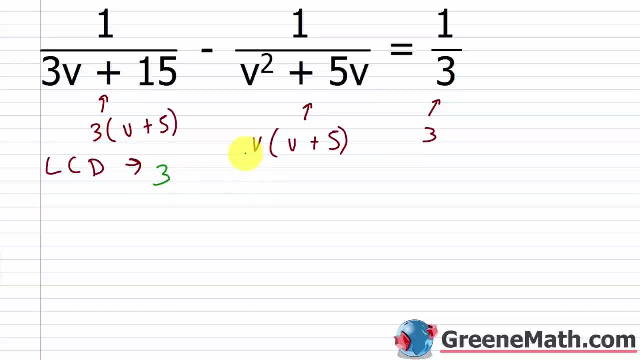 I just have a three, So it looks like I have a three here and here, So that goes in the LCD. I have a v And then I have a v plus five. Let's erase all this And I think I might be able to fit this on the screen. 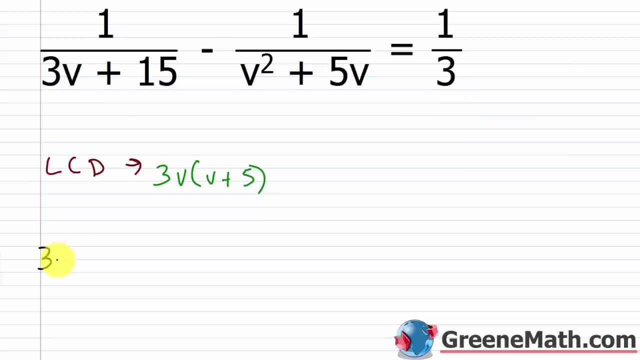 So let's try that. So I would have three v Times the quantity v plus five Times One over three v plus fifteen Minus One over v squared plus five v, And then equals- And let me just scroll down and get a little room going- 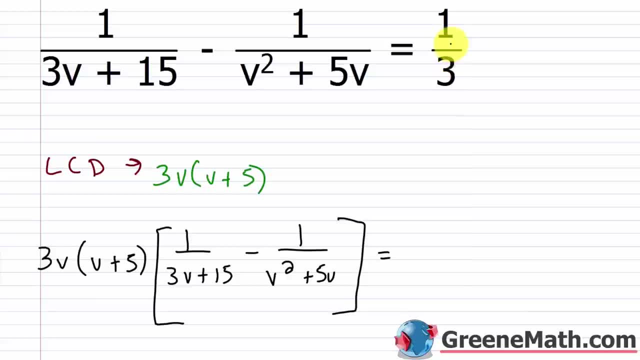 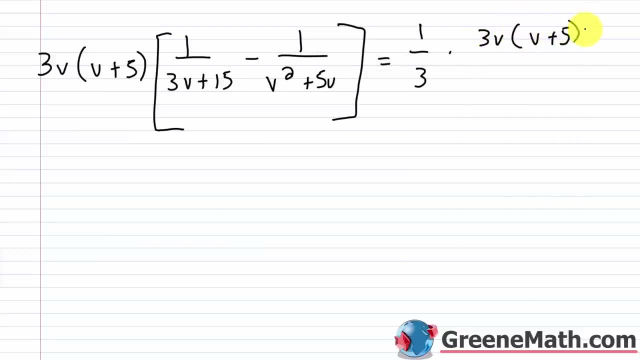 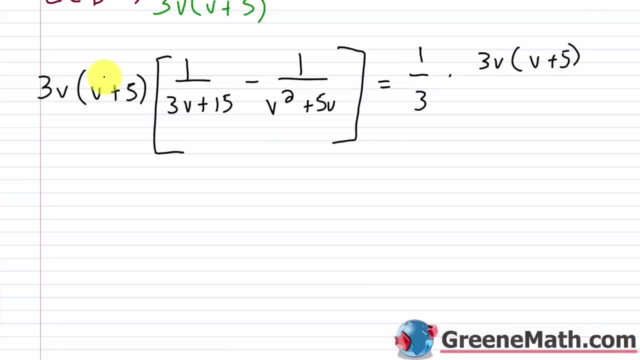 We have one third there, So one third Times three v plus fifteen Times three v Times the quantity v plus five. Okay, So we fit that on the screen Now. what I'm going to do here Is I'm going to be using my distributive property. 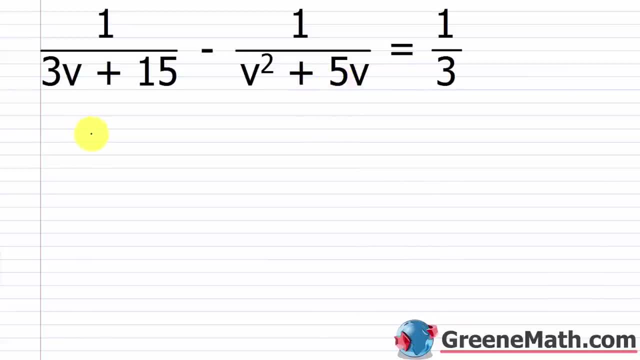 is equal to one third so again I'm looking for the LCD and for this guy I've got to factor it it can factor into three times the quantity v plus five for this guy I can factor out a v and I have v plus five and for this guy I just have a three it looks like I have a three here and here so that goes in the LCD I have a v and then I have a v plus five so my LCD is three v times the quantity v plus five let's erase all this 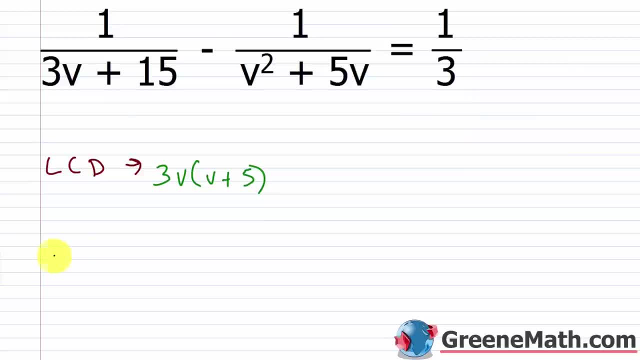 and I think I might be able to fit this on the screen so let's try that so I would 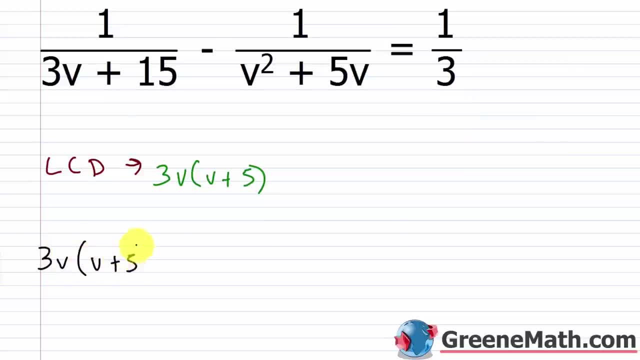 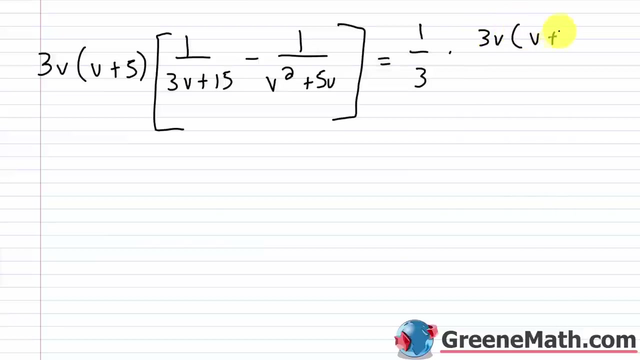 have three v times the quantity v plus five times one over three v plus fifteen minus one over v squared plus five v and then equals and let me just scroll down and get a little room going we have one third there so one third times three v times the quantity v plus five okay 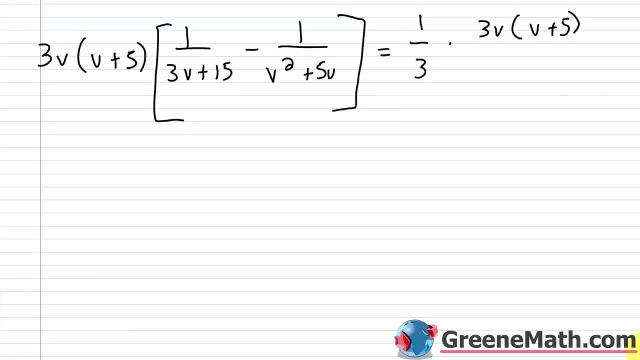 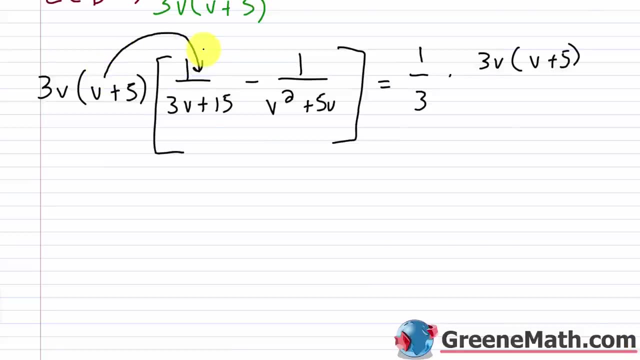 so we fit that on the screen now what I'm going to do here is I'm going to be using my distributive property and I'm going to distribute this to this so if I have three v plus fifteen again that's three times the quantity v plus five if I factor it the v plus five would cancel with this and the three would cancel with this so essentially I have v times one which is just v now let me kind of erase what I cancelled there and do this 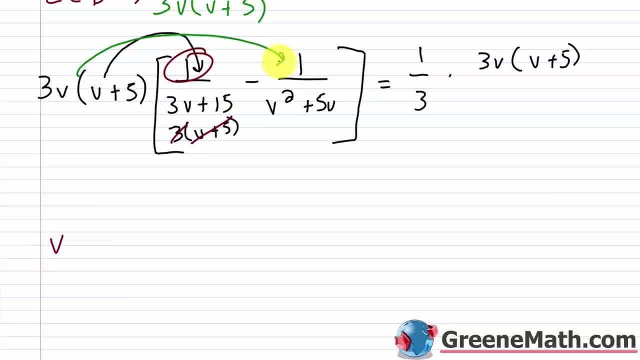 again we're going to use our distributive property over here now in factored form this is v times the quantity v plus five so in this particular case the v is going to cancel and the v plus five is going to cancel so that's gone and what I'm left with is three times one or just minus three so then minus three and then over here 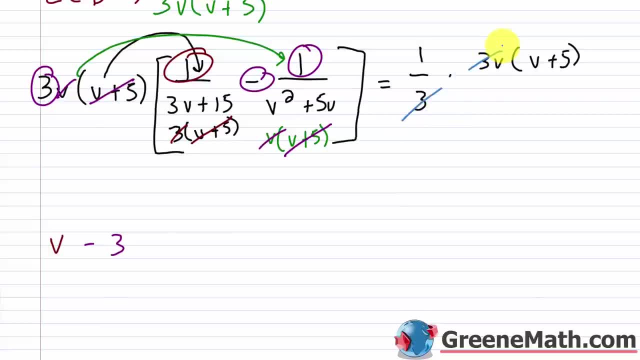 if I look only a three is going to cancel so I'm left with equals v times the quantity v plus five 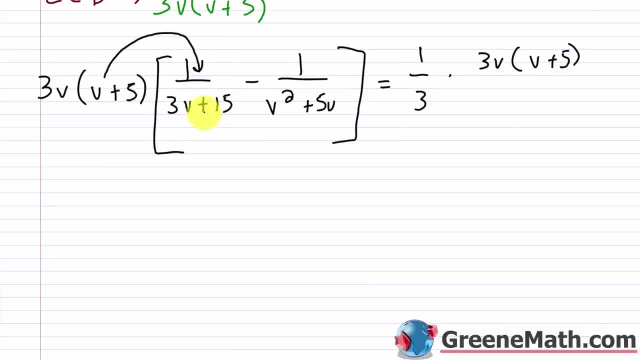 And I'm going to distribute this to this. So if I have three v plus fifteen, Again, that's three times the quantity v plus five. If I factor it, The v plus five Would cancel with this And the three would cancel with this. 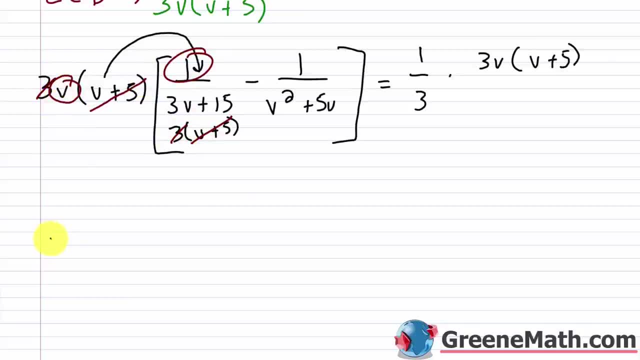 So essentially I have V times one. Now let me kind of Erase what I cancelled there And do this again. We're going to use our distributive property over here Now in factored form. this is V times the quantity v plus five. 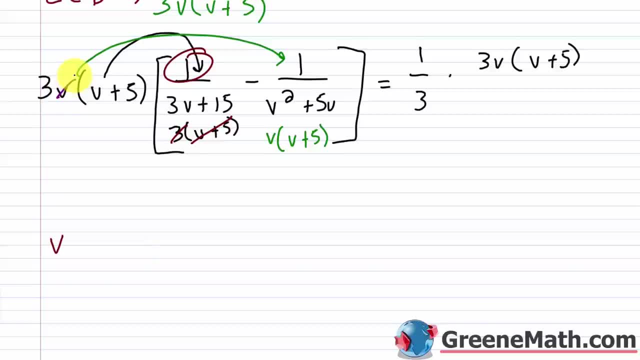 So in this particular case, The v is going to cancel And the v plus five is going to cancel. So that's gone, And what I'm left with is three times one Or just minus three. So then minus three And then over here. 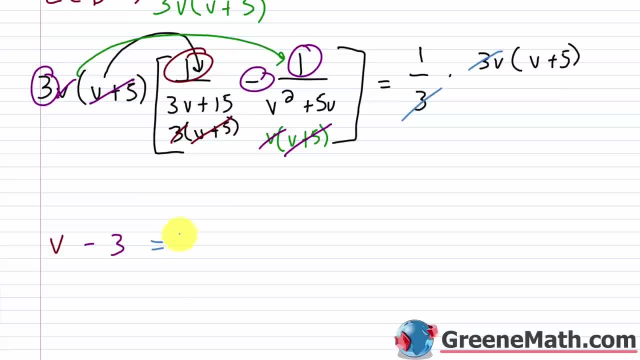 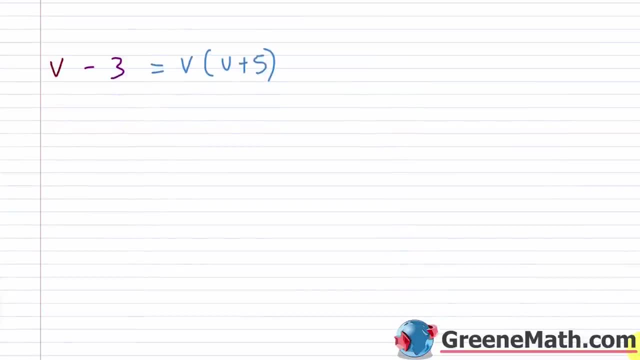 If I look, only a three is going to cancel. So what I'm left with? Equals v times the quantity v plus five. Okay, So we've got it In kind of a simple form. It won't take us very long to solve this now. 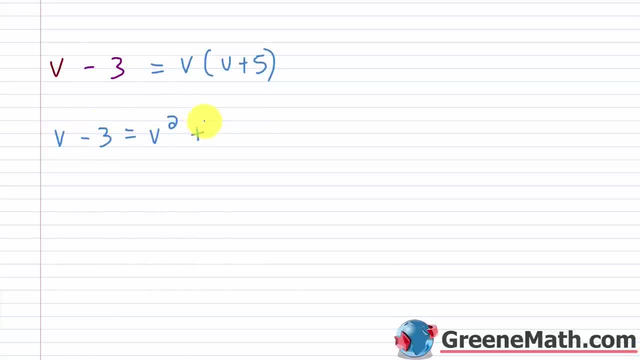 We have: v minus three is equal to V times v is v squared Plus v times five is five v. Okay, so now What I want to do? I want to subtract v away from each side of the equation And I want to add: 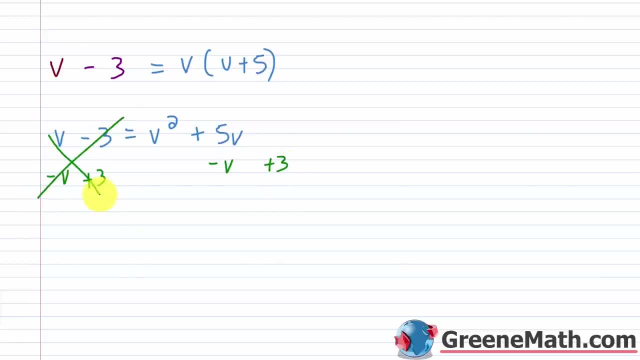 Three to both sides of the equation. So that's going to cancel itself out. So I'm going to have: zero is equal to V squared Plus four, v Plus three. Now we have this set up as a quadratic equation. We cannot solve quadratic equations. 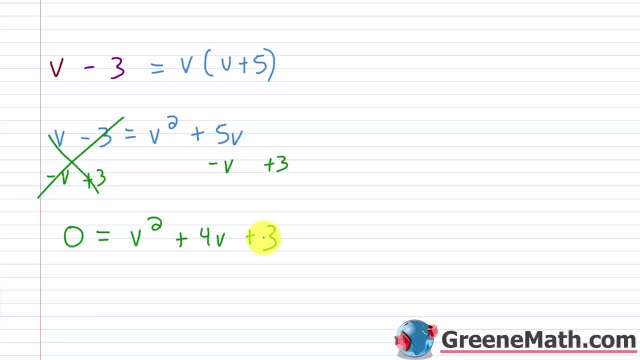 That we can't factor, Because I haven't taught you how to do it yet, Unless you know how to do it from outside of my course. There is something called The quadratic formula And, completing the square That we're going to get to at the very end of algebra one. 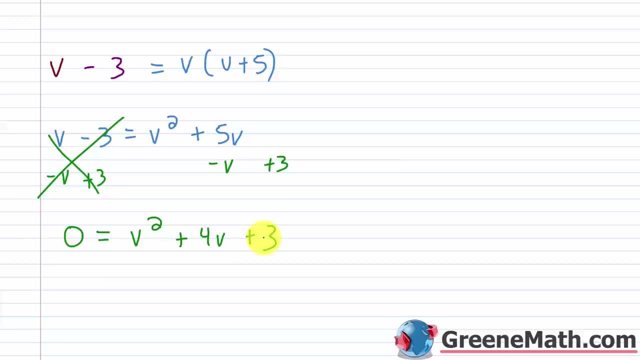 So until we get to that point, Unless we can factor this, We can't solve it. But fortunately I gave you a problem that you can do, So this is going to factor into one Two integers whose sum is four And whose product is three. 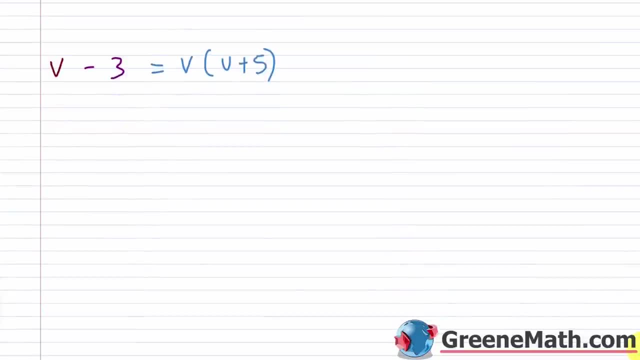 okay so we've got it in kind of a simple form it won't take us very long to solve this now we have v minus three is equal to v times v is v squared plus v times five is five v okay so now what I want to do I want to subtract v away from each side of the equation and I want to add three to both sides of the equation so that's going to cancel itself out so I'm going to have zero is equal to v squared plus four v 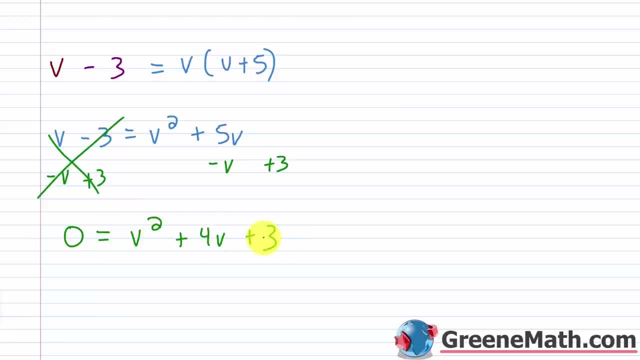 plus three now we have this set up as a quadratic equation we cannot solve quadratic equations that we can't factor because I haven't taught you how to do it yet unless you know how to do it from outside of my course there is something called the quadratic formula and completing the square that we're going to get to at the very end of algebra one so until we get to that point unless we can factor this we cannot solve it but fortunately I gave you a problem that you can do so this is going 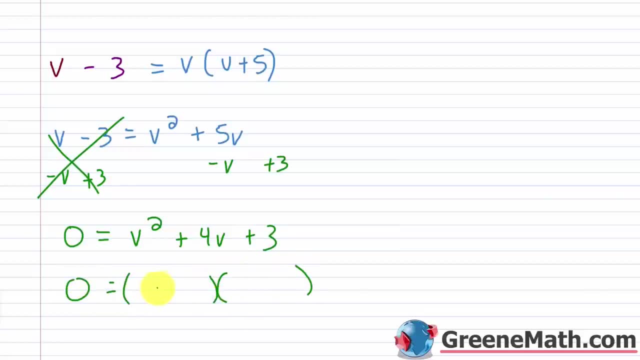 to factor into one two integers whose sum is four and whose product is three that's three and one 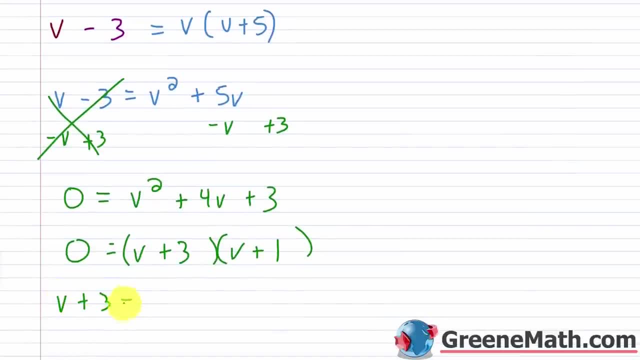 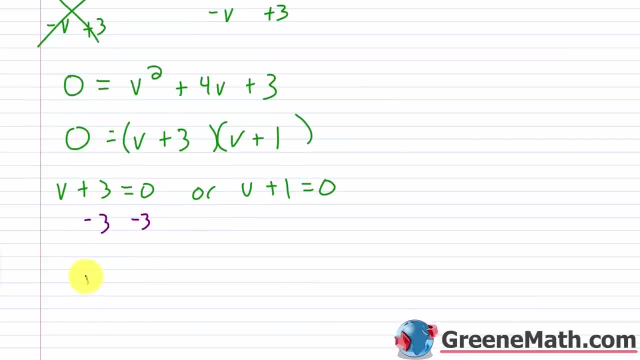 so I would get that v plus three is equal to zero or v plus one is equal to zero so solving that I just subtract three away from each side here I get v is equal to negative three and then over here I subtract one away I get v is equal to negative one so here are my two proposed 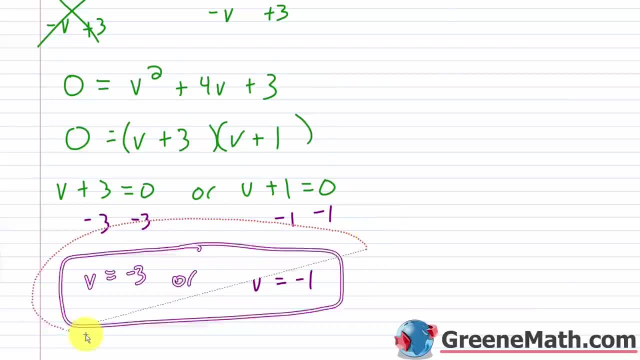 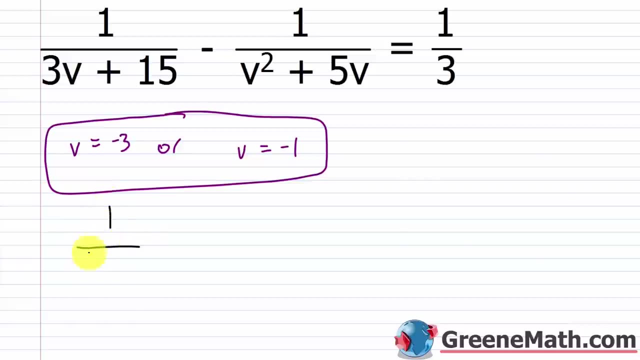 solutions let's go back up and check them okay so let's check each one separately and so I'm going to do one over let's start with negative three so three times negative three is negative nine and negative nine plus fifteen is six then my minus I've got one over v squared negative three squared would be nine and then five v five times negative three is negative fifteen so nine minus fifteen would be negative six so this would 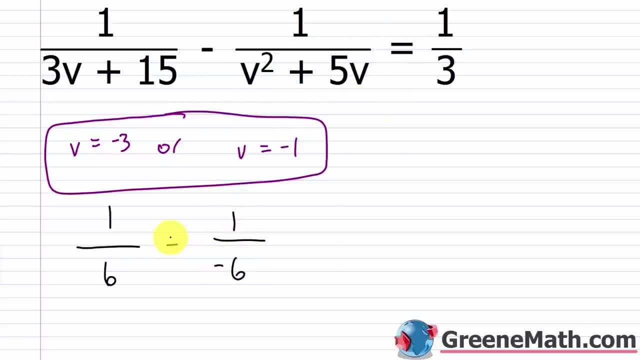 be minus a negative one sixth so this is plus positive one sixth 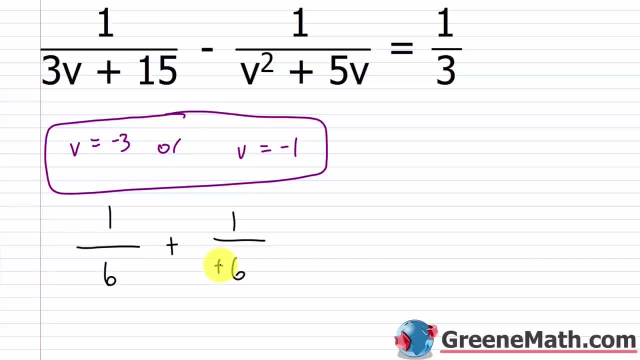 so essentially we could write this as what two over six which is one third so this is one third 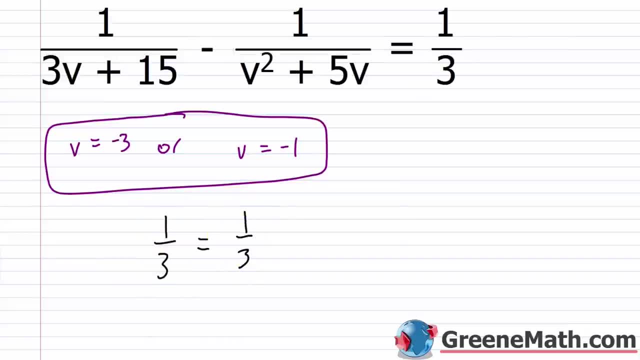 and this says one third over here so this one checks itself out 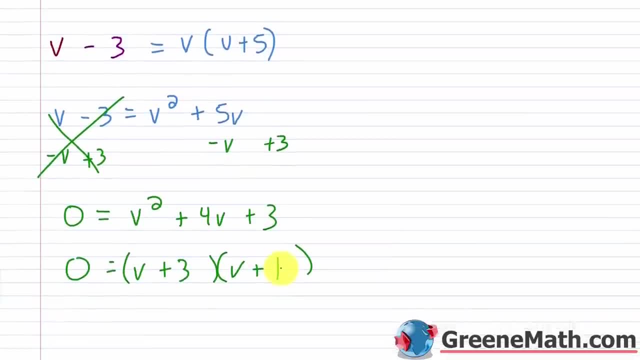 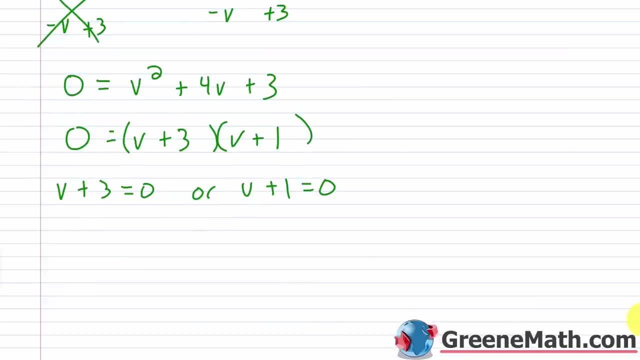 That's three and one, So I would get that V plus three is equal to zero, Or V plus one is equal to zero. So solving that, I just subtract three away from each side. here I get v is equal to negative three. 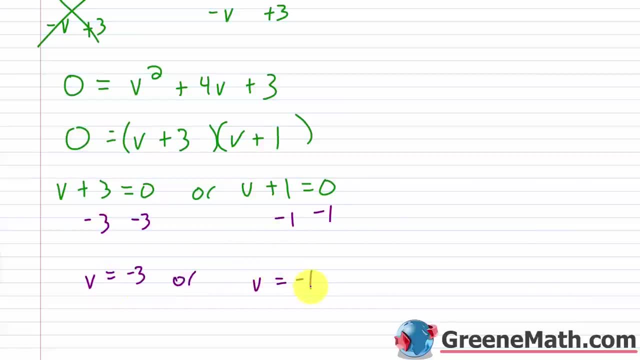 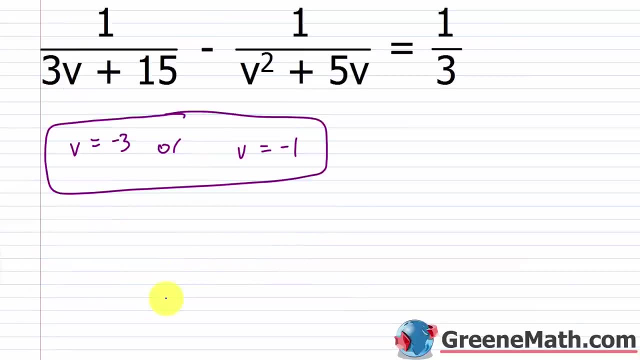 And then over here I get: v is equal to negative one. So here are my two Proposed solutions. Let's go back up and check them, Okay. so let's check each one separately, And so I'm going to do One over. 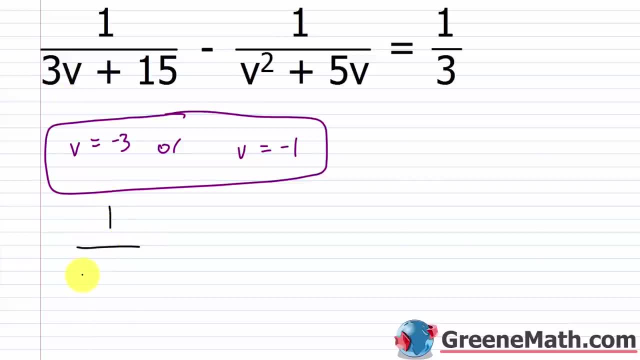 Let's start with negative three. So three times negative. three is negative nine And negative nine plus fifteen is six. Then minus, I've got one over V squared. Negative three squared would be nine And then five v. So nine minus fifteen would be negative six. 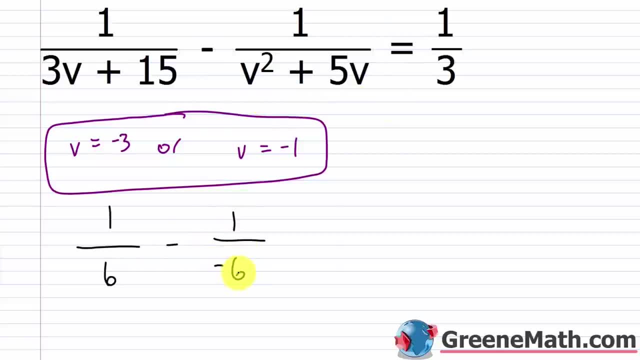 So this would be minus a negative One sixth. So this is plus positive one sixth. So essentially we could write this as: What? Two over six, Which is one third. So this is one third And this says one third over here. 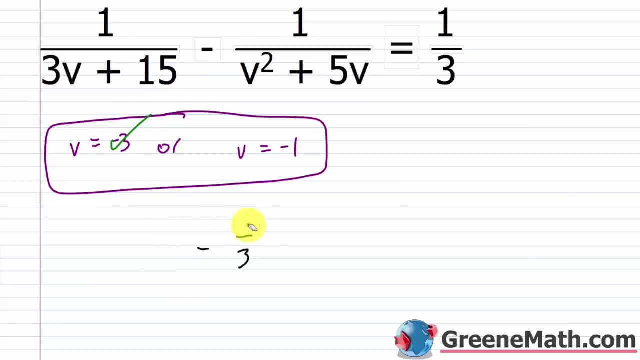 So this one checks itself out. This is good to go. So now let's try negative one. This is negative three. Negative three plus fifteen is twelve. So this is one over twelve And then minus. I'm going to have one over. 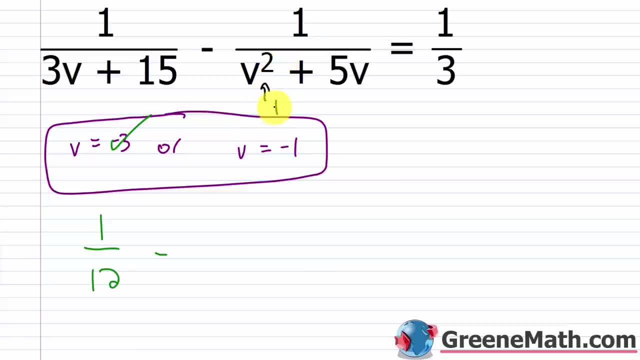 V squared Negative. one squared is one, So this would be one Five times negative. one is negative five, So one minus five Is negative four. So I'd have minus a negative one. fourth. Now This is plus a positive, So this is going to. 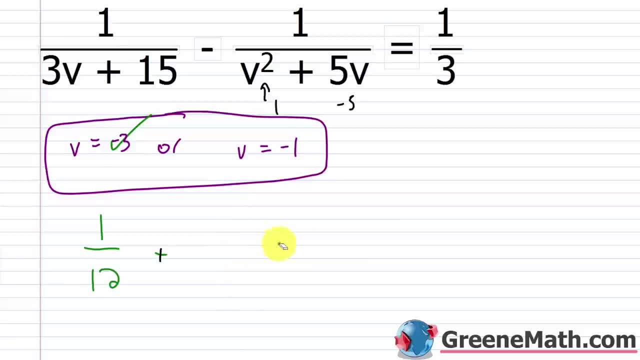 Multiplying by three over three. So this is going to be three twelfths, So three twelfths. Now, if I Add one and three, I get four. So this is four twelfths. And what is four twelfths reduced to? 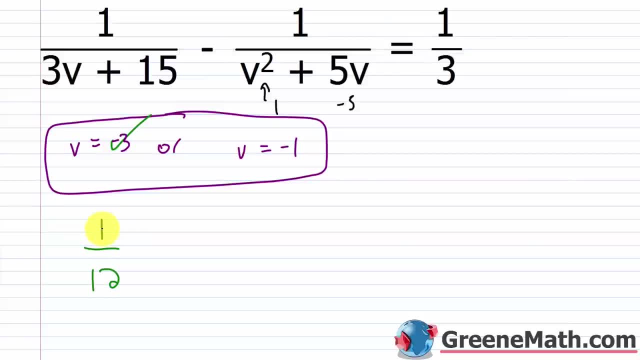 It reduces to one third. Four divided by four is one. Twelve divided by four is three. So I get one third equals One third from over there. So again, we've found the big winner. So v can equal negative three And v can equal negative one. 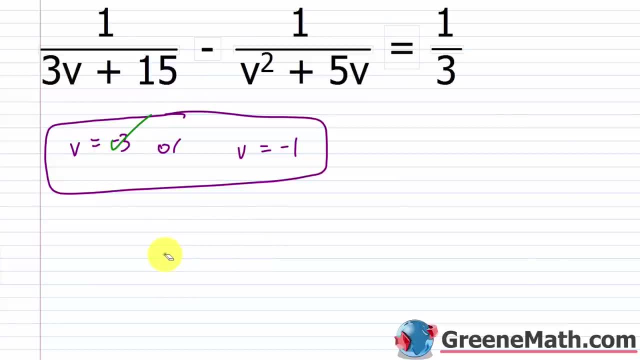 this is good to go so now let's try negative one 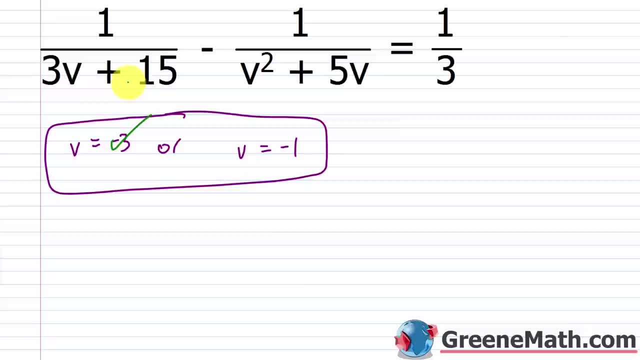 so three times negative one is negative three negative three plus fifteen is twelve so this is one over twelve and then minus 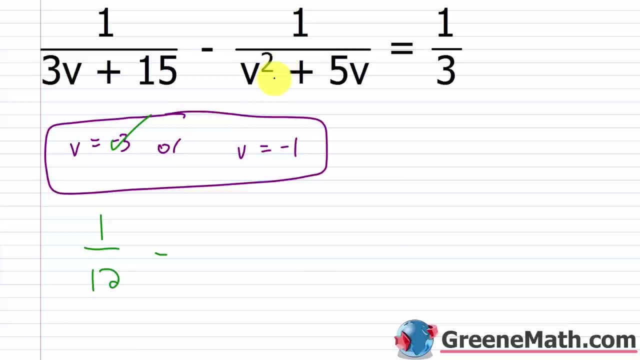 I'm going to have one over v squared negative one squared is one so this would be one five times negative one is negative five so one minus five is negative four so I'd have minus a negative one fourth now this is plus a positive and I could change this into multiplying by three over three so this is going to be three twelfths so three twelfths 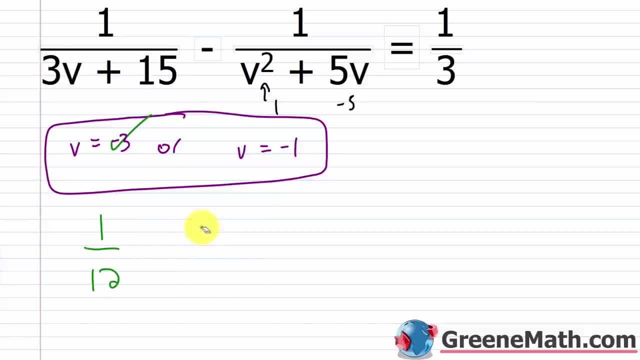 now if I add one and three I get four so this is four twelfths and what is four twelfths reduced to it reduces to one third four divided by four is one twelve divided by four is three so I get one third equals one third from over there 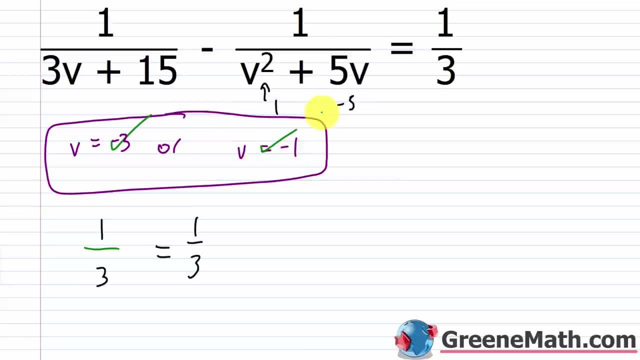 so again we've found the big winner so v can equal negative three or v can equal negative 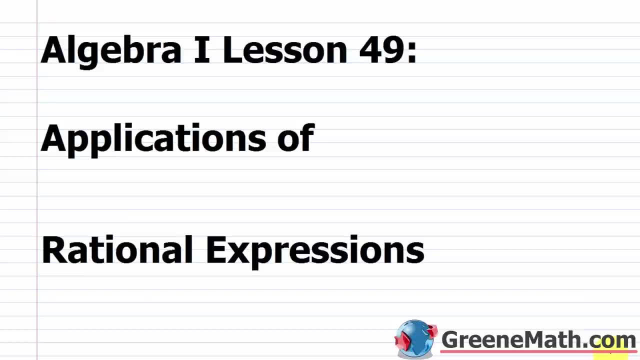 one hello and welcome to algebra one lesson forty nine in this video we're going to learn about applications of rational 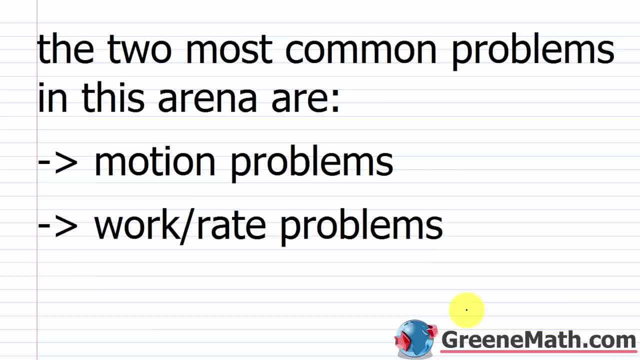 expressions so in this video basically what we're going to be doing is looking at some word problems that require equations with rational expressions now the two most common problems in this arena are going to be motion word problems which we saw back at the beginning of algebra one use your distance formula there distance is equal to rate of speed times the amount of time traveled and then something that's new to us is going to be these work rate problems or some people say rate of work problems 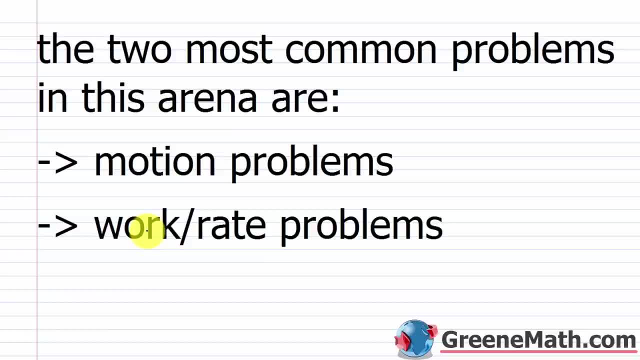 so these are really really easy to solve and we're going to get to them at the very end 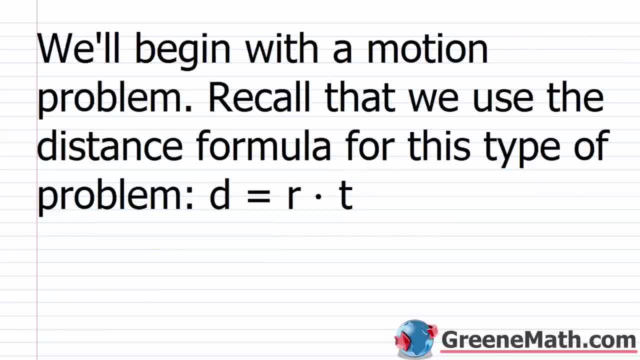 alright so we're going to begin today with a motion word problem so I want you to recall that we used the distance 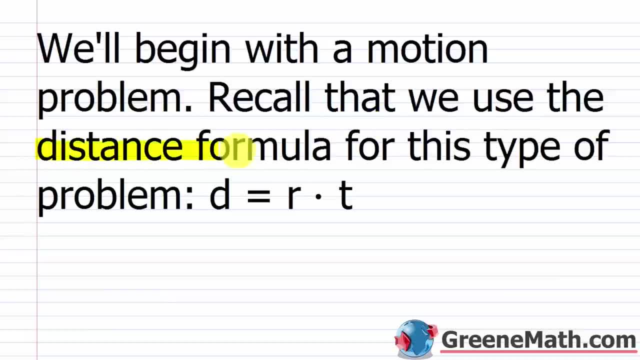 formula let me just highlight that real quick the distance 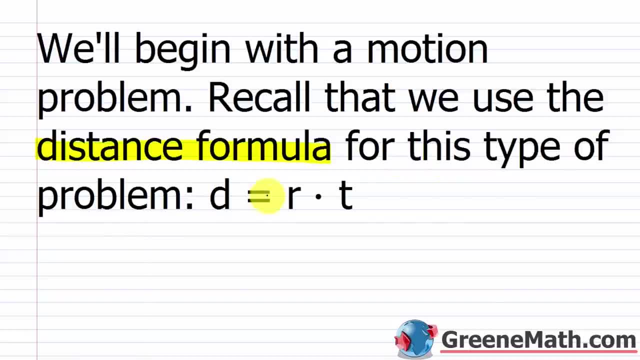 formula for this type of problem so we have d is equal to r times t remember this d stands for distance 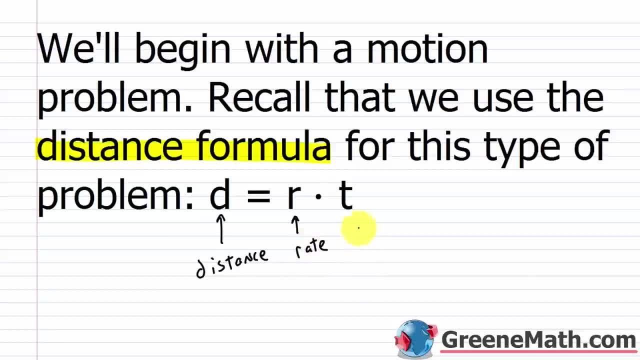 the r stands for rate of speed and t stands for time 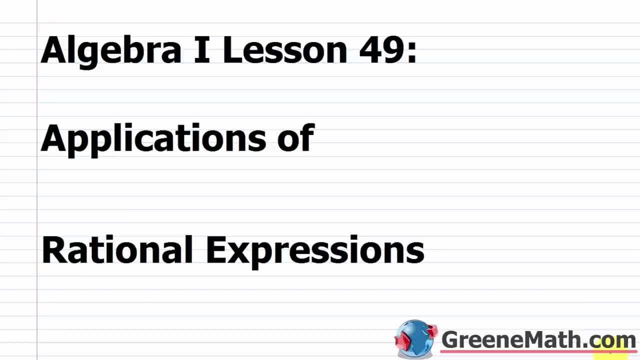 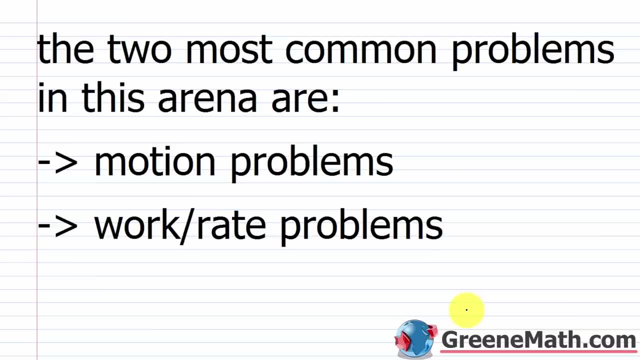 Hello and welcome to algebra one, Lesson forty nine. In this video we're going to learn about Applications of rational expressions. So in this video, Basically what we're going to be doing Is looking at some word problems That require equations with rational expressions. 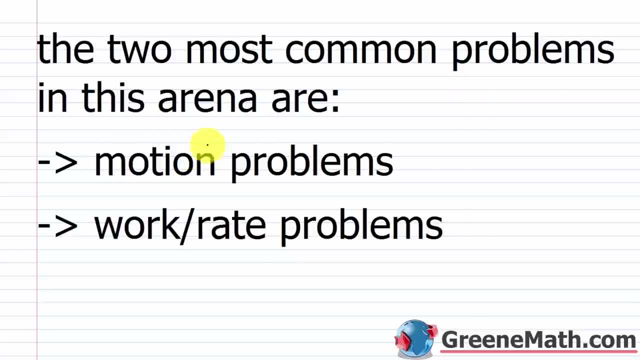 Now, the two most common Problems in this arena Are going to be motion word problems, Which we saw back at the beginning of algebra one. Use your distance formula there. Distance is equal to rate of speed Times, the amount of time traveled. 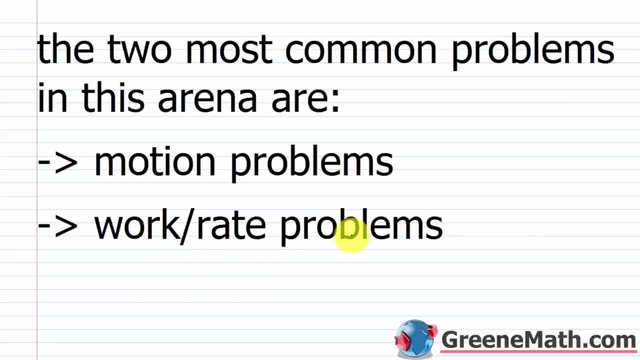 And then something that's new to us Is going to be these work rate problems, Or some people say rate of work problems. So these are really really Easy to solve. We're going to get to them at the very end of the lesson. 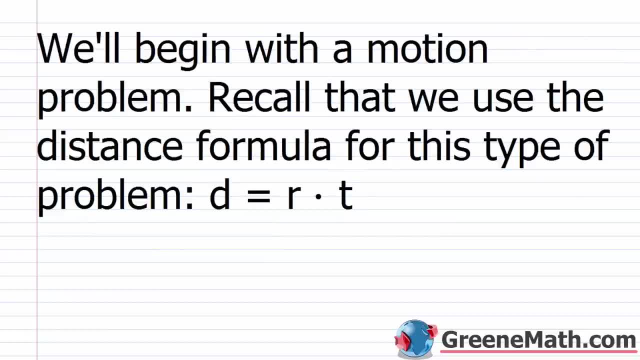 Alright, so we're going to begin today With a motion word problem, So I want you to recall that We used the distance formula. Let me just highlight that real quick: The distance formula for this type of problem. So we have: D is equal to r times t. 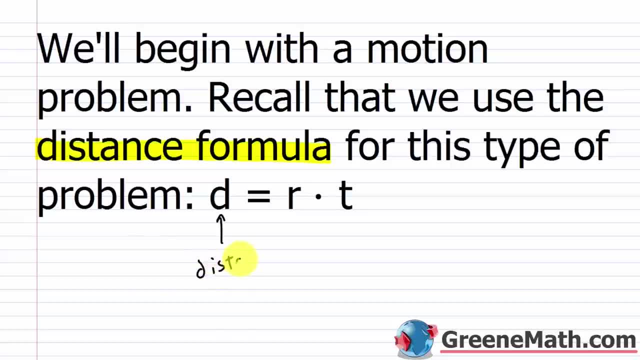 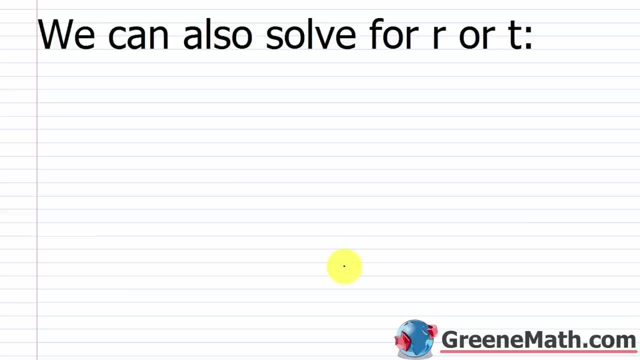 Remember this: d stands for distance, The r stands for Rate of speed And t stands for Time traveled. So something that's going to be new for us here Is that we're going to manipulate the distance formula And we're going to be solving it. 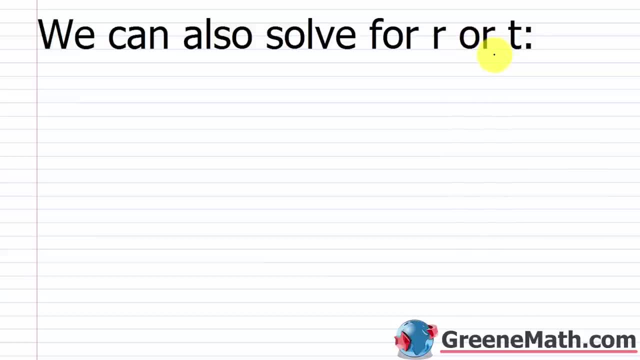 For r or t. So, for example, if I have Distance is equal to Rate times time, And I want to Solve this for the rate, Let me highlight that. How would I go about doing that? Well, all we're going to do is realize: 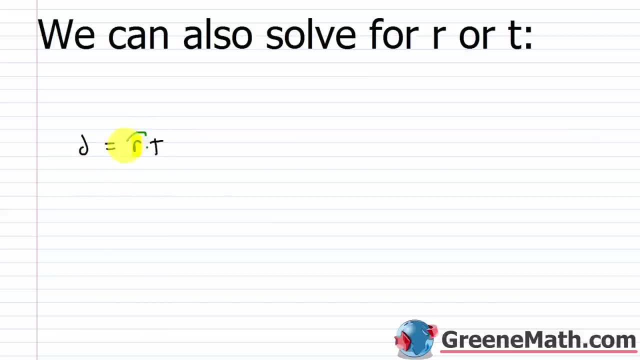 That if t is multiplying r To get r by itself, I just divide both sides of the equation By t And what's going to happen is The t is going to cancel here and here And on the right side of the equation. 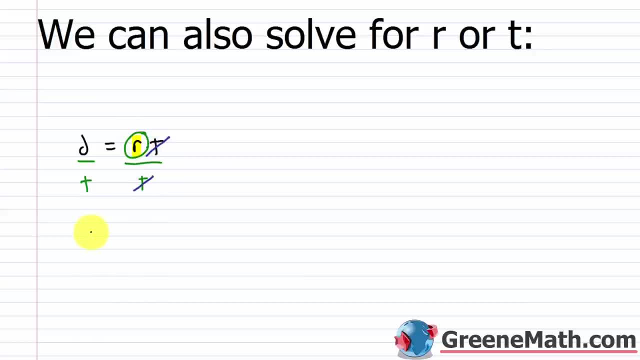 I'm just left with r. It's isolated, And so what I have is I have distance over time. Now let's check that real quick And make sure that that makes sense. We know from the traditional Distance formula That if I am going, 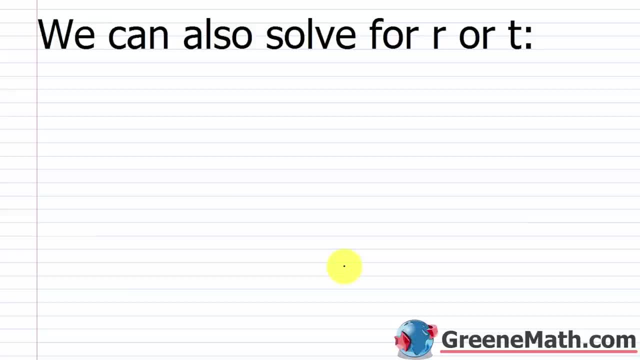 traveled so something that's going to be new for us here is that we're going to manipulate the distance formula and we're going to be solving it for r or t so for example if I have distance is equal to rate times time and I want to solve this for the rate let me highlight that how would I go about doing that well all we're going to do is realize that if t is multiplying r to get r by itself 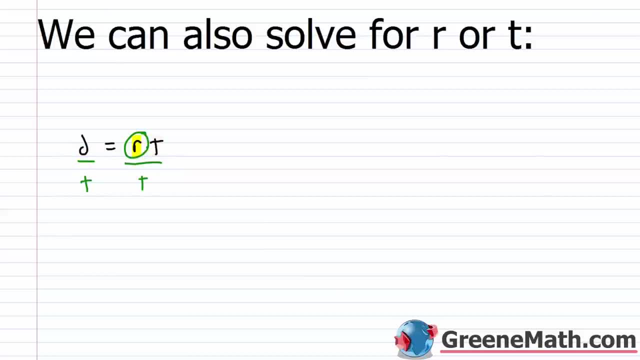 I just divide both sides of the equation by t and what's going to happen is the t is going to cancel here and here and on the right side of the equation I'm just left with r it's isolated and so what I have is I have distance over time is equal to rate now let's check that real quick 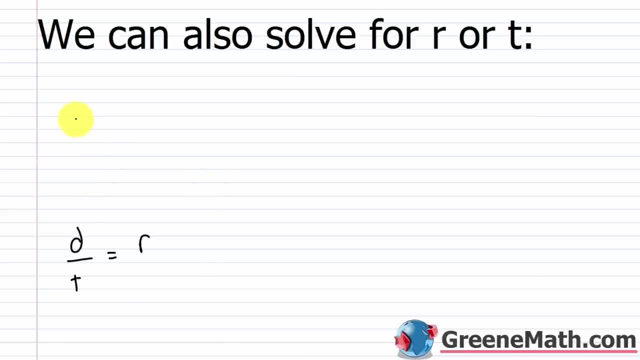 and make sure that that makes sense we know from the traditional distance formula 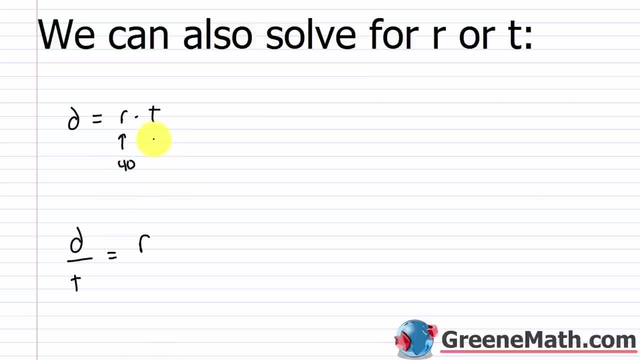 that if I am going let's say 40 miles per hour and I do this for 3 hours 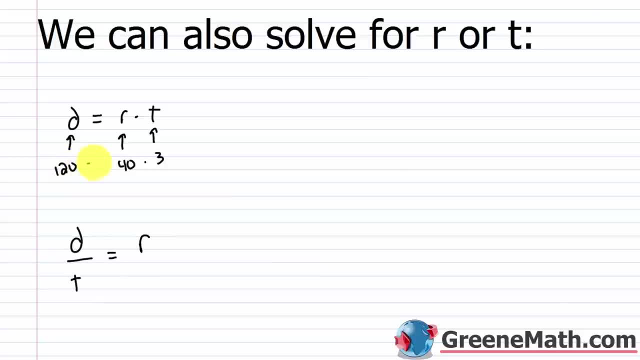 40 times 3 is 120 I've traveled 120 miles ok so that makes sense if I plug in the same numbers here is that going to work so if I plug in 120 here and I plugged in a 3 here would I get 40 here well yes I would 120 divided by 3 is in fact 40 right so we're good to go there 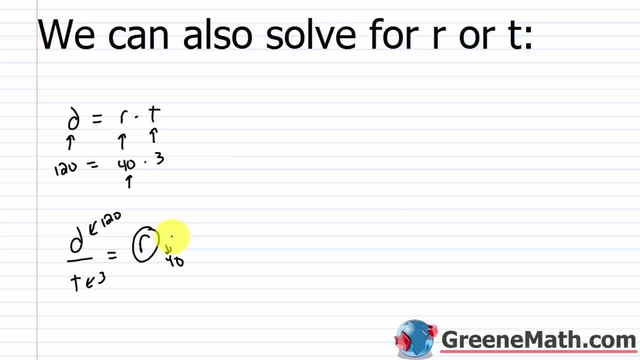 now the other thing we might have to solve for is time so if I have distance is equal to rate times time 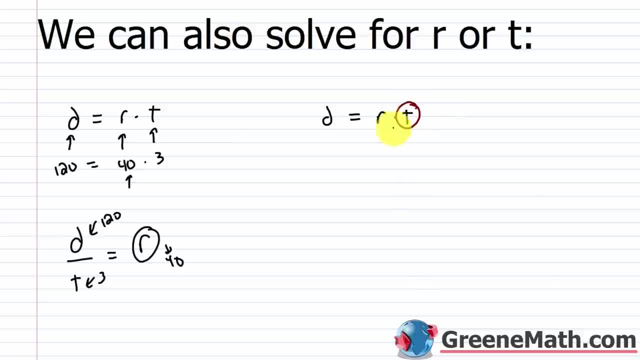 I'm going to use the same logic to solve for time I want to isolate this guy so I'm going to divide both sides of the equation by r so I can isolate the t let's cancel this with this I'm going to be left with time is equal to distance over rate and again you can say ok using this example if I plugged in 120 here and I plugged in a 40 there 120 divided by 40 is in fact 3 so we're good to go 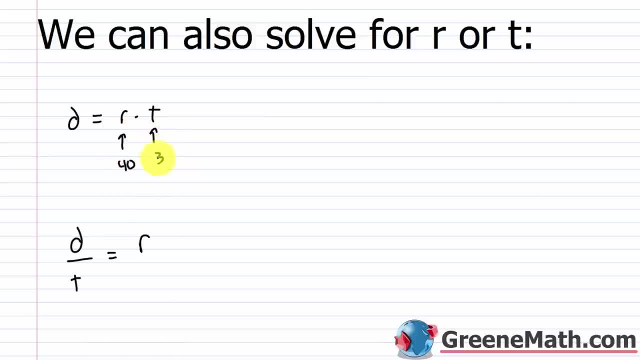 Let's say 40 miles per hour And I do this for 3 hours. 40 times 3 is 120.. I've traveled 120 miles. Okay, so that makes sense. If I plug in the same numbers here, Is that going to work? 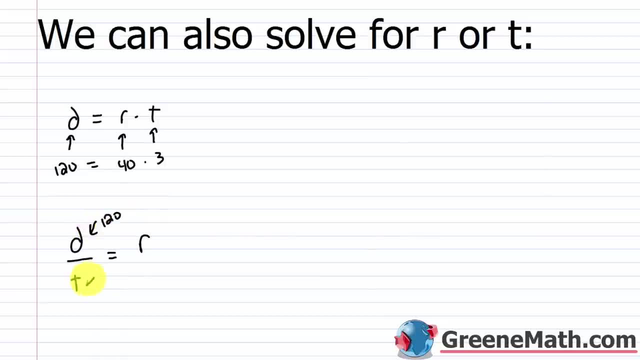 So if I plugged in 120 here And I plugged in a 3 here, Would I get 40 here? Oh, yes, I would. 120 divided by 3 is in fact 40.. Right, so we're good to go there. 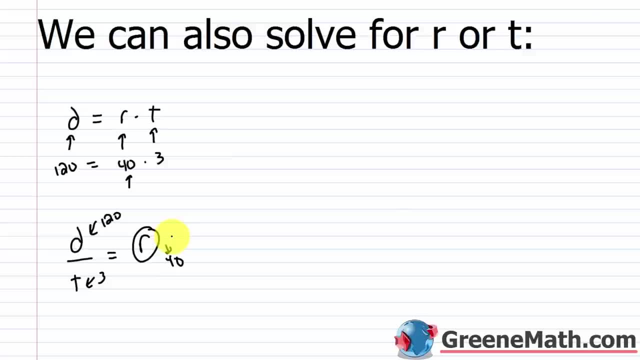 Now The other thing we might have to solve for is time. So if I have distance Is equal to rate times, time, I'm going to use the same logic To solve for time. I want to isolate this guy, So I'm going to divide both sides of the equation by r. 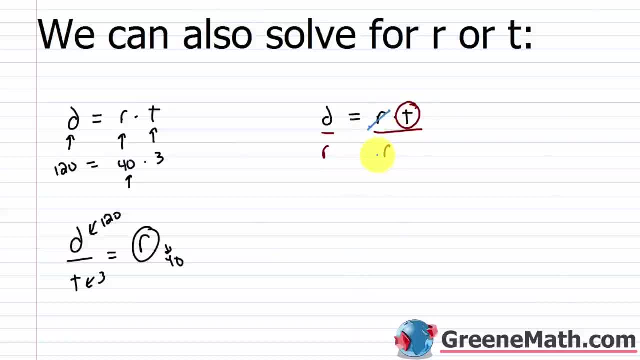 So I can isolate the t. Let's cancel this with this And I'm going to be left with. Time is equal to distance over time, Over rate, And again you can say okay, Using this example, If I plugged in 120 here. 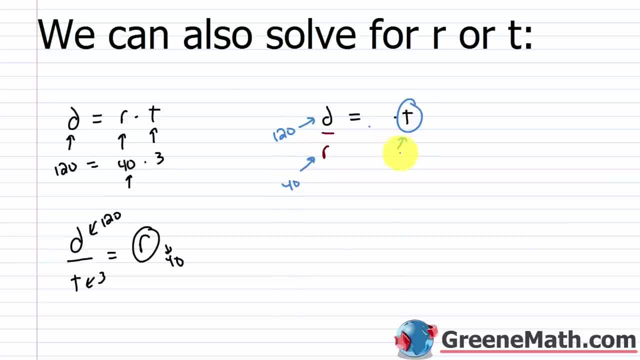 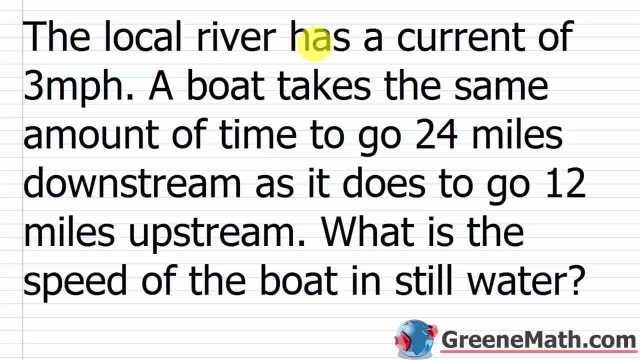 And I plugged in a 40 there. 120 divided by 40 is in fact 3.. So we're good to go. Alright. so let's go ahead and take a look at the first problem. So the local river Has a current of 3 miles per hour. 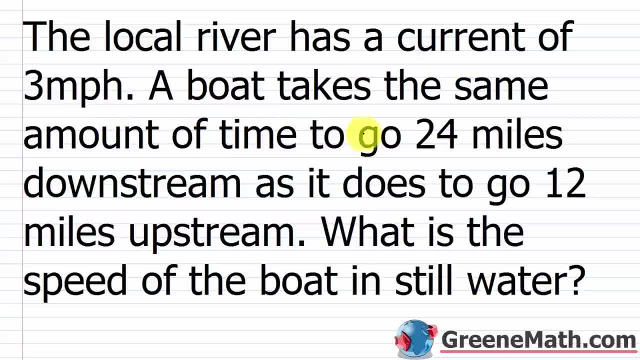 A boat takes The same amount of time to go 24 miles downstream. Okay, that's going with the current. In case you don't know that, We're going to go 12 miles upstream, Upstream is against the current. What is the speed of the boat? 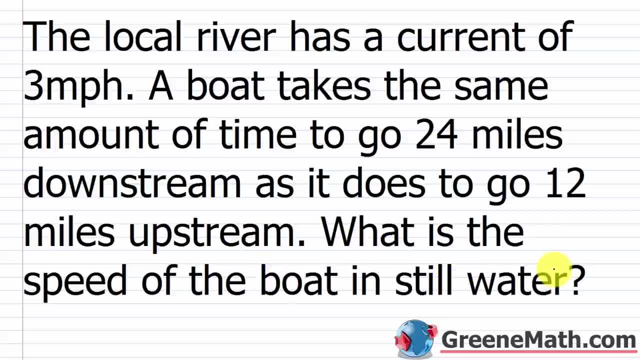 In still water. So it might seem like This is a difficult problem, But it's really not. Let's go ahead and make a little table To kind of organize our information. The two things we're going to think about is The scenario where we're going downstream. 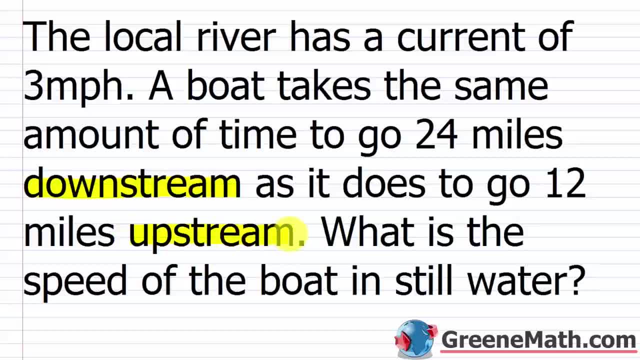 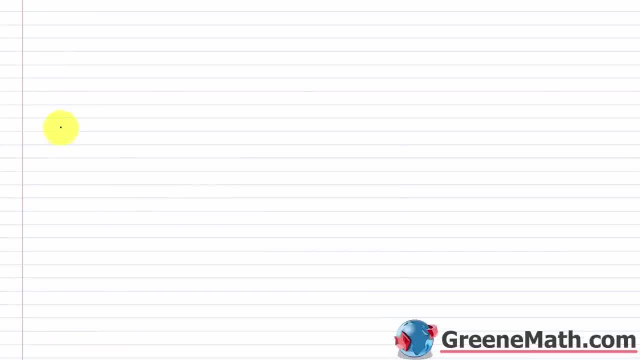 Again, that's with the current And the scenario where we're going to go upstream And that's against the current. Let's scroll down here real quick, So we'll kind of think about: Okay, we have upstream And we have downstream. 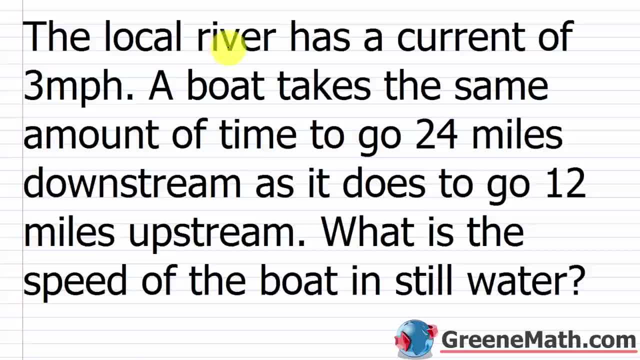 alright so let's go ahead and take a look at the first problem so the local river has a current of 3 miles per hour a boat takes the same amount of time to go 24 miles downstream going with the current as it does to go 12 miles upstream upstream is against the current what is the speed of the boat in still water so it might seem like this is a difficult problem but it's really not let's go ahead and make a little table 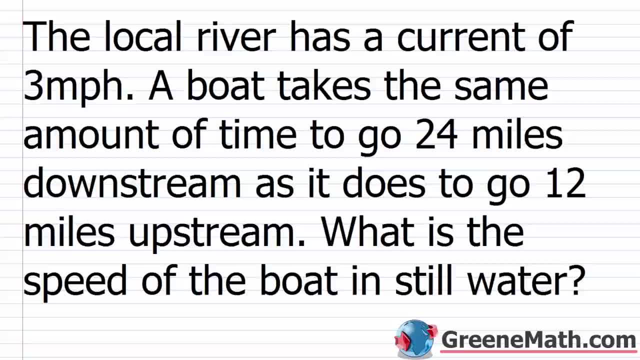 to kind of organize our information the two things we're going to think about is the scenario where we're going downstream again that's with the current and the scenario where we're going to go upstream and that's against the current 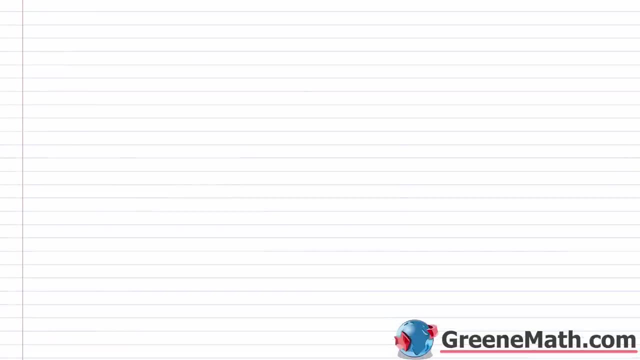 let's scroll down here real quick so we'll kind of think about ok we have upstream and we have downstream 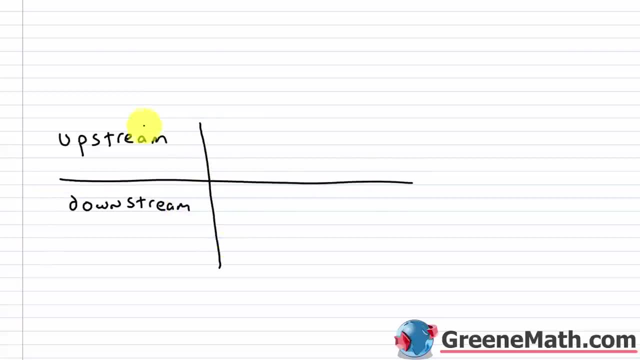 ok so let me just draw a little line here now the components of the distance formula let's think about those 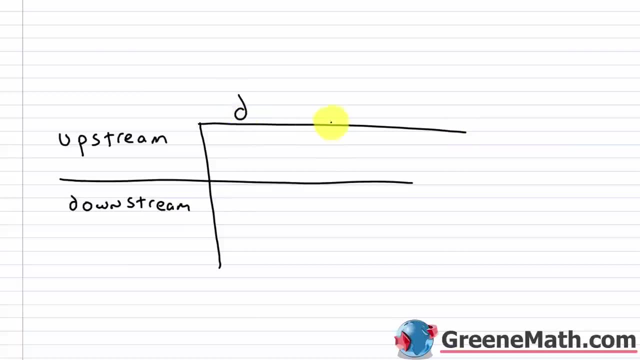 so we have distance so I'm just going to abbreviate with a D we have speed which I'm going to use an R for and then we have the time so what I want to do here is just fill in this table and 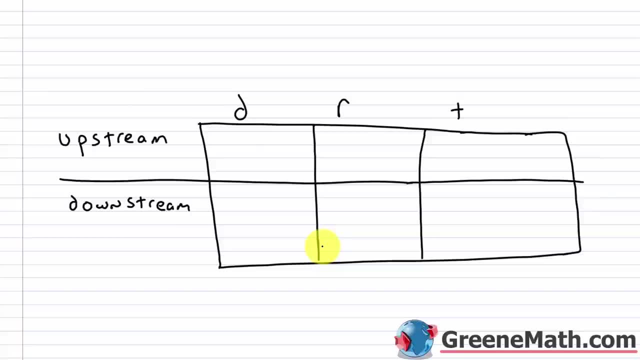 get the information that I'm going to need to create an equation that's going to allow me to solve and figure out an answer for this problem 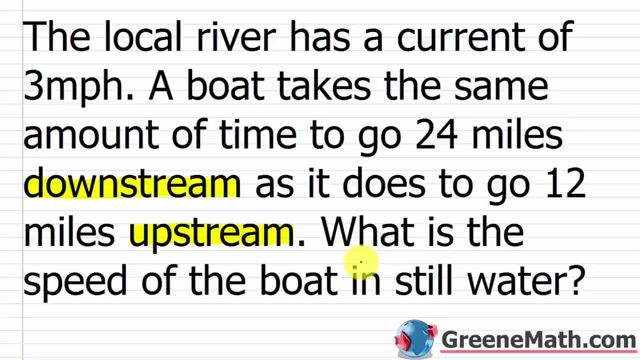 let's scroll back up to the top real quick so it tells us in the problem 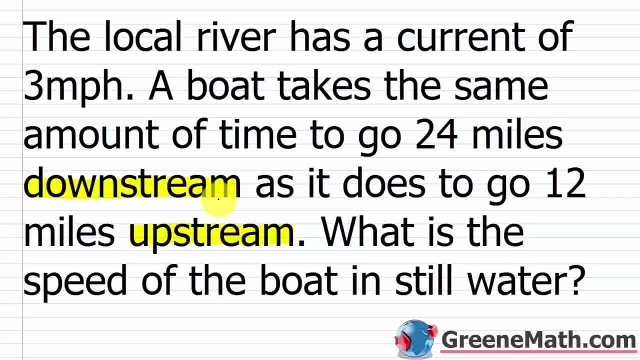 that the boat is going 24 miles downstream in the same amount of time as it does to go 12 miles upstream 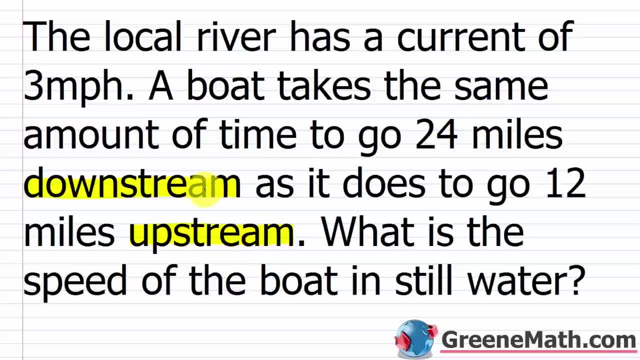 so for the distance I'm going to put 24 miles under downstream and 12 miles under upstream ok so I'm going to write 12 here and 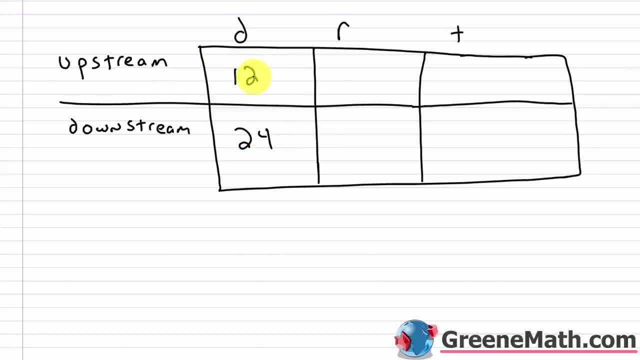 24 here again the distance when I'm going upstream is 12 miles the distance when I'm going downstream is 24 miles 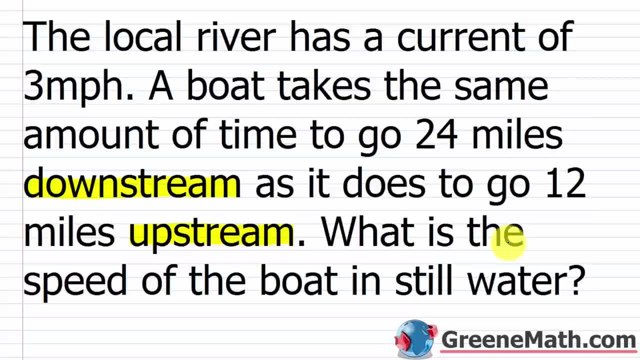 now let's think about the rate so when we think about the rate of speed 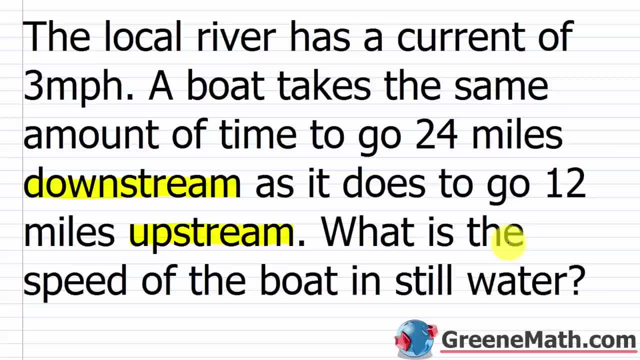 again this is how fast we're traveling the only information we're really given 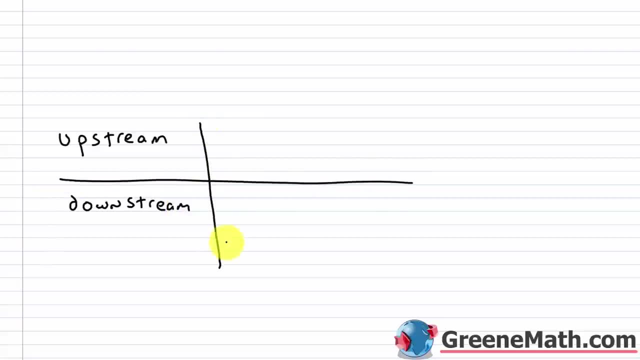 Okay, so let me just draw a little line here. Now, the components of the distance formula. Let's think about those. So we have distance, Which I'm just going to abbreviate with a D. We have The rate of speed, Which I'm going to use an R for. 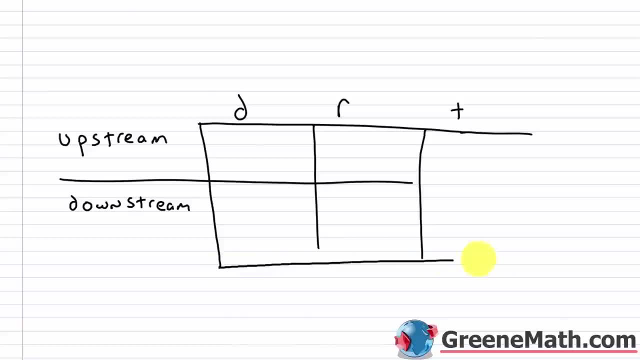 And we have the time. So what I want to do here Is just fill in this table And get the information that I'm going to need To create an equation That's going to allow me to solve And figure out an answer. 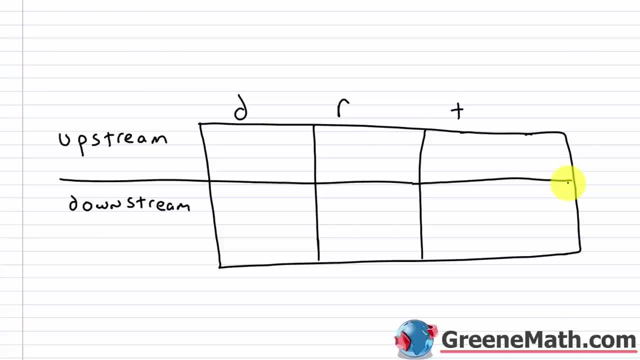 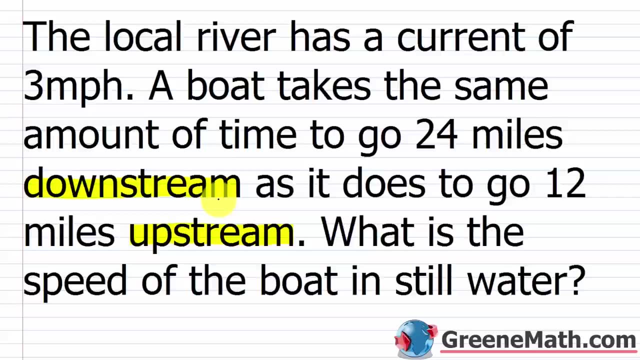 For this problem. Let's scroll back up to the top real quick, Alright. so it tells us in the problem That the boat is going 24 miles downstream In the same amount of time as it does To go 12 miles upstream. 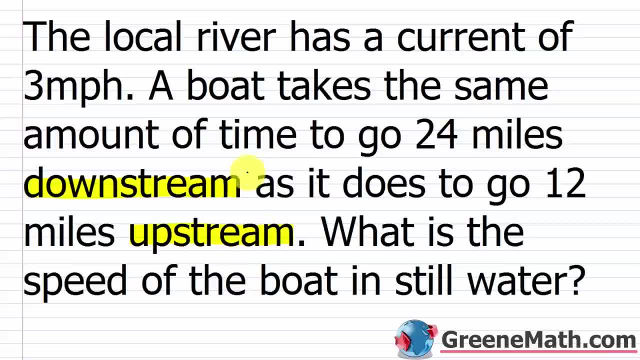 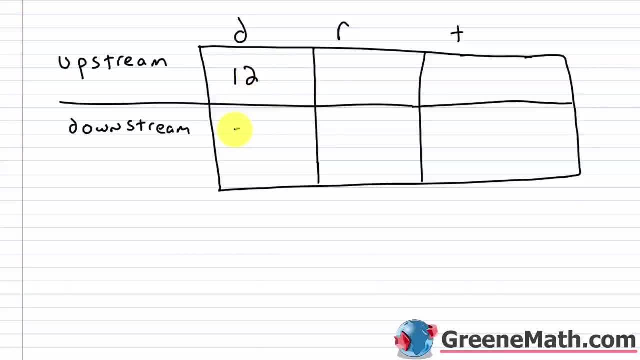 So for the distance, I'm going to put 24 miles Under downstream And 12 miles under upstream. Okay, so I'm going to write 12 here And 24 here. Again, the distance when I'm going upstream Is 12 miles. 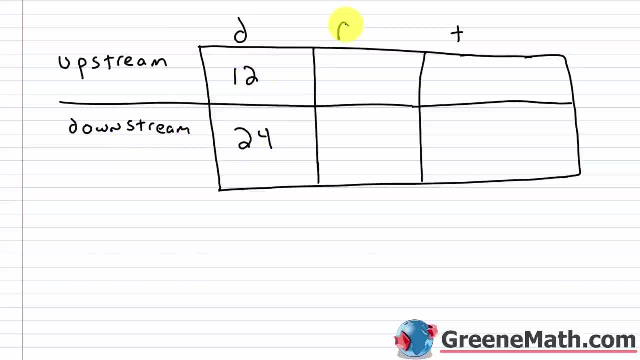 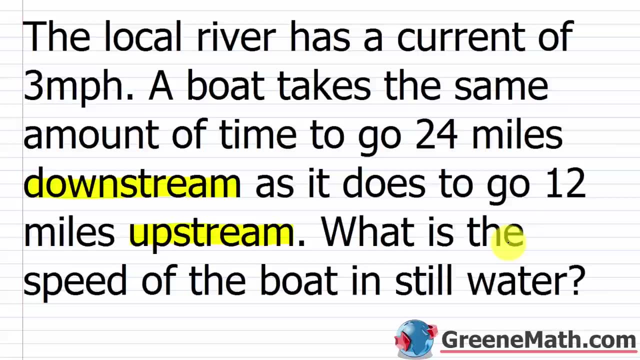 The distance when I'm going downstream Is 24 miles. Now let's think about the rate. So when we think about the rate of speed- Again, this is how fast we're traveling- The only information we're really given Is that the local river has a current of 3 miles per hour. 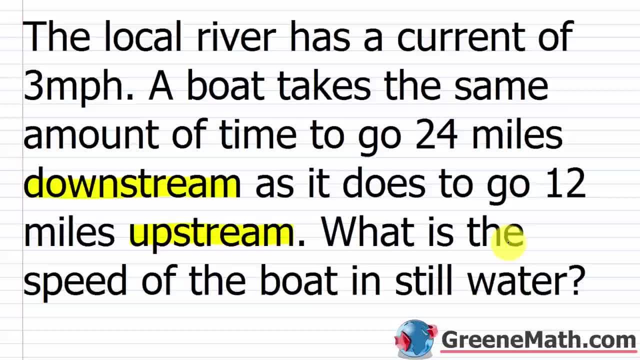 Now what you're supposed to know here Is that If you're going upstream, You are fighting the current. So whatever the amount of speed you're going In- miles per hour, Like if you're going in still water- You've got to subtract 3 away from that. 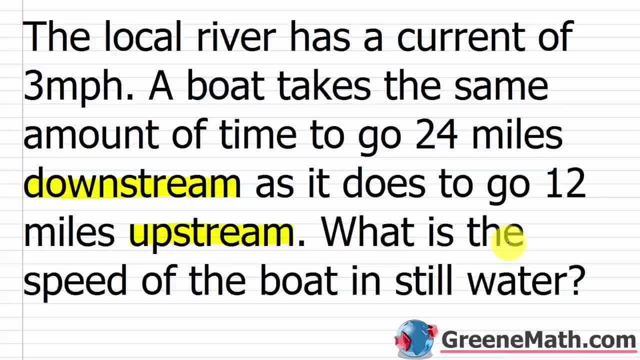 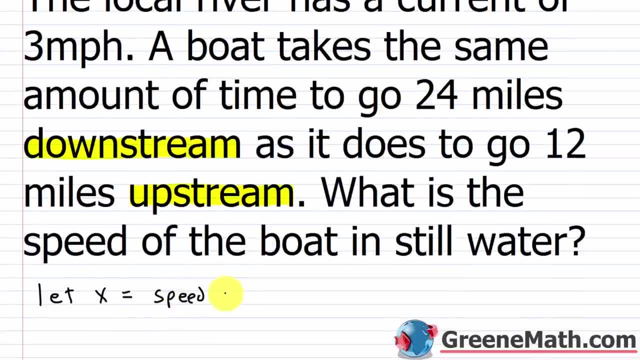 Because you're fighting the current. So if I let a variable Like x- Let's say let x equal the speed Of the boat In still water- Well, what would happen is The speed when I'm going upstream Would be x. 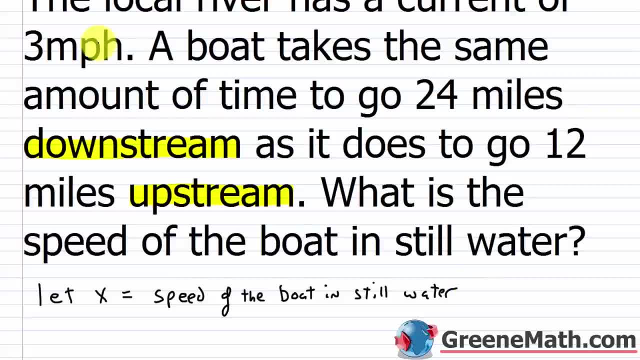 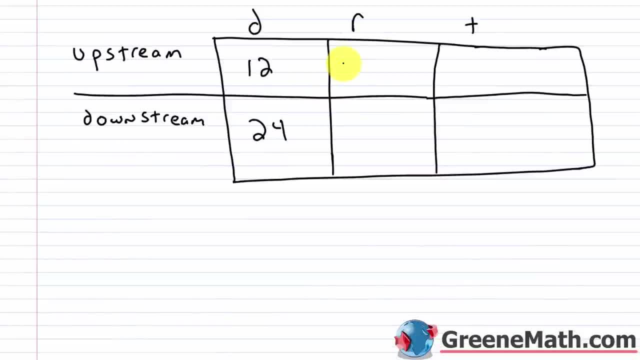 The speed of the boat in still water Minus 3.. Because that's the speed of the current And that's what I'm fighting. So let's scroll down and put that So again, for the upstream speed It's going to be x. 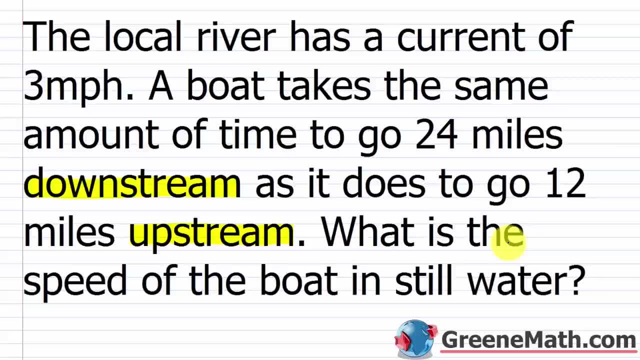 is that the local river has a current of 3 miles per hour doesn't give us any other information now what you're supposed to know here is that if you're going upstream you are fighting the current so whatever the amount of speed 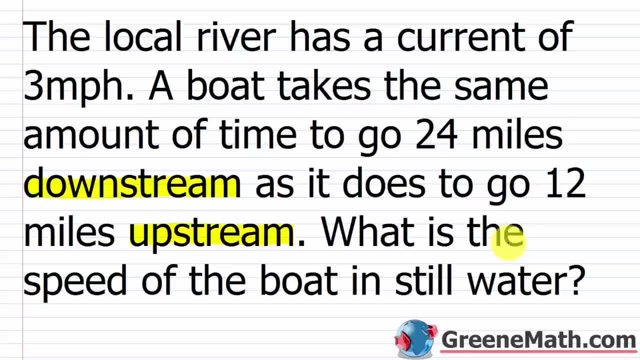 you're going in miles per hour like if you're going in still water you've got to subtract 3 away from that because you're fighting the current 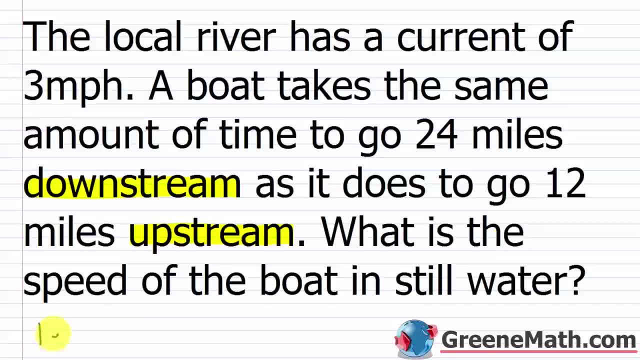 so if I let a variable like x 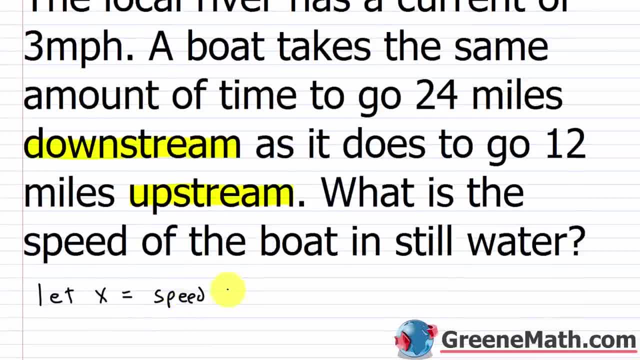 let's say let x equal the speed of the boat in still water 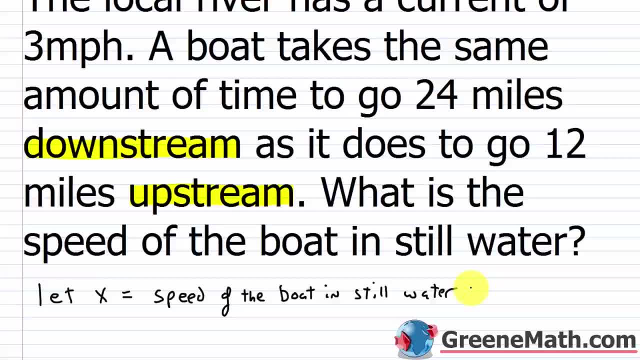 well what would happen is the speed when I'm going upstream would be x the speed of the boat in still water minus 3 because that's the speed of the current and that's what I'm fighting 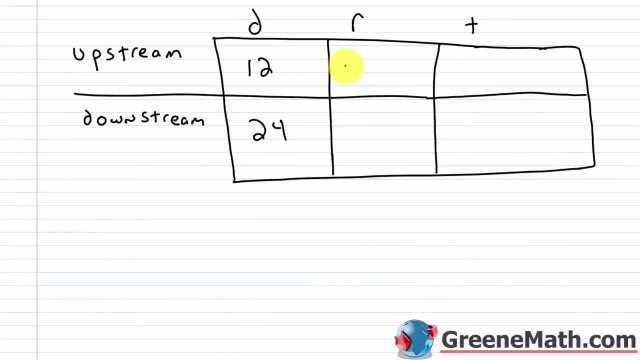 so let's scroll down and put that so again for the upstream speed it's going to be x the speed of the boat in still water 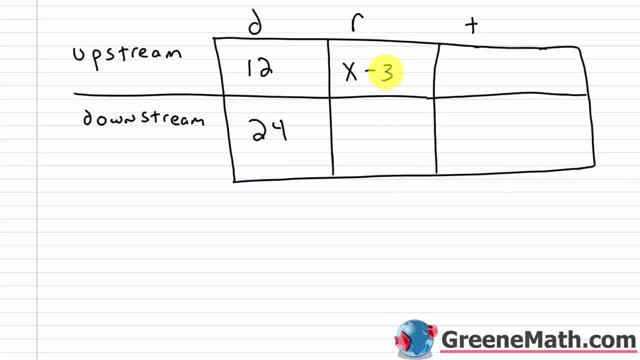 minus 3 the speed of the current and then for the downstream speed 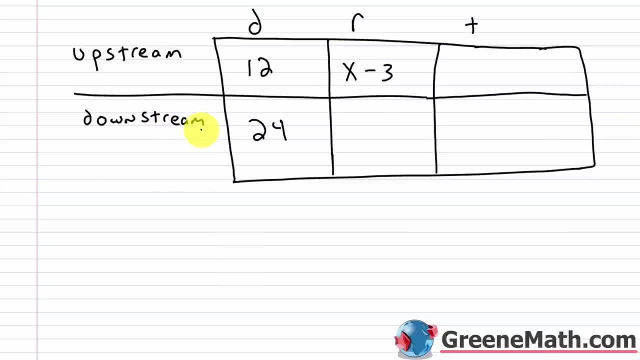 it's just as easy we think about the speed of the boat in still water as x and then now if I'm going downstream that means I'm going with the current so the current is pushing on my boat it's making me go faster by 3 miles per hour so I would add 3 to that x so x plus 3 is the speed of the boat going downstream x minus 3 is the speed of the boat going upstream now how do I go about getting a time? 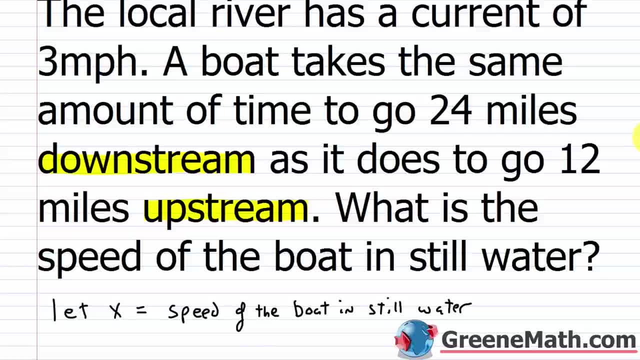 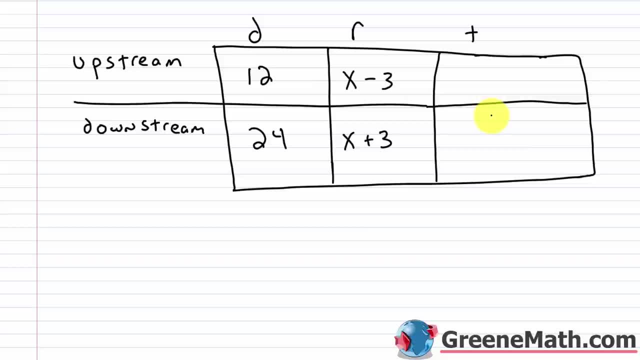 looking back through the problem the only thing it really says about the time is that it takes the same amount of time to go 24 miles downstream as it does to go 12 miles upstream so what I can do here as we talked about a little while ago is I can get a time for each one and then I can set those times equal to each other so let's take that one step at a time 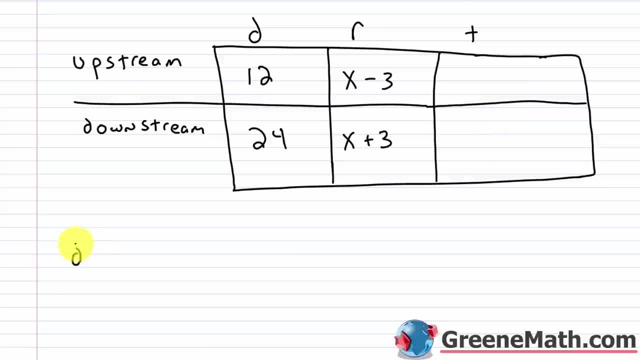 to get a time remember the d equals r times t can be solved for t 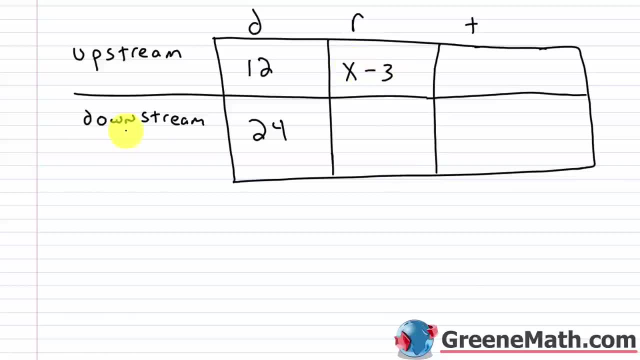 The speed of the boat in still water Minus 3.. The speed of the current Right we think about the speed of the boat In still water is x. And then now, if I'm going downstream, That means I'm going with the current. 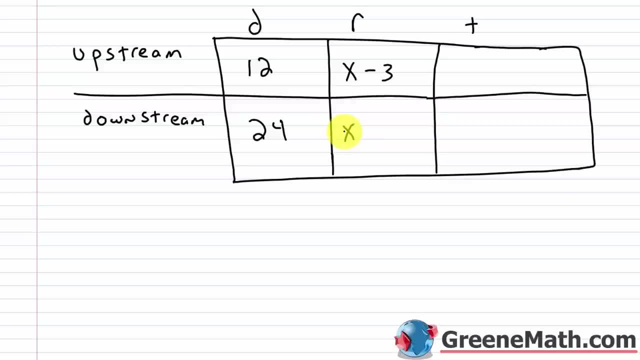 So the current is pushing on my boat. It's making me go faster By 3 miles per hour, So I would add 3. To that x. So x plus 3 is the speed Of the boat going downstream. x minus 3 is the speed of the boat. 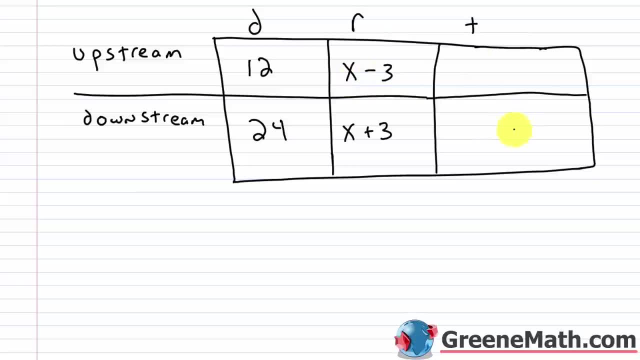 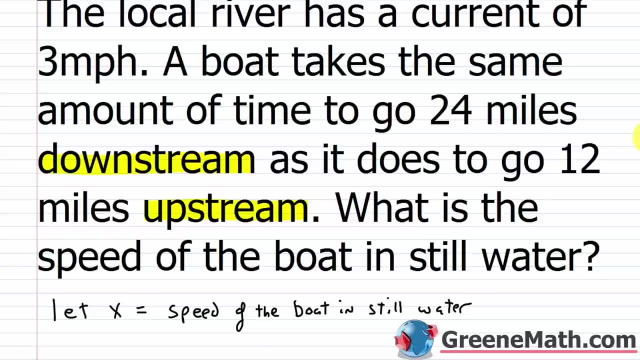 Going upstream. Now, how do I go about getting a time? Well, reading back through the problem, The only thing it really says about the time Is that it takes the same amount of time to go 24 miles downstream As it does to go 12 miles upstream. 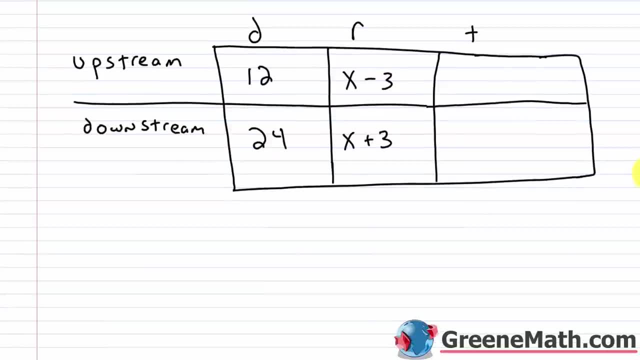 So what I can do here, As we talked about a little while ago, Is I can get a time For each one, And then I can set those times equal to each other. So let's take that one step at a time To get a time. 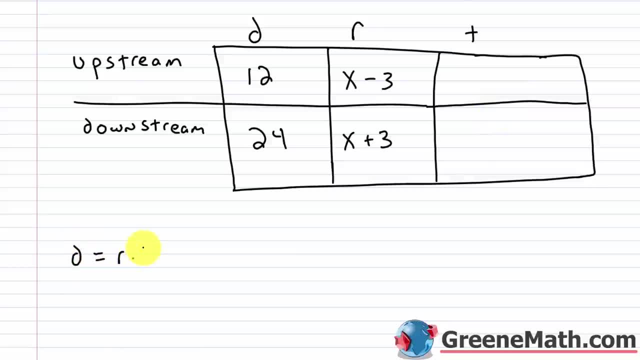 Remember the d Equals r times. t Can be solved for t. So if I divide both sides of the equation By r to isolate t, As we did earlier, This cancels with this And I've got t by itself. So time is equal to distance over rate. 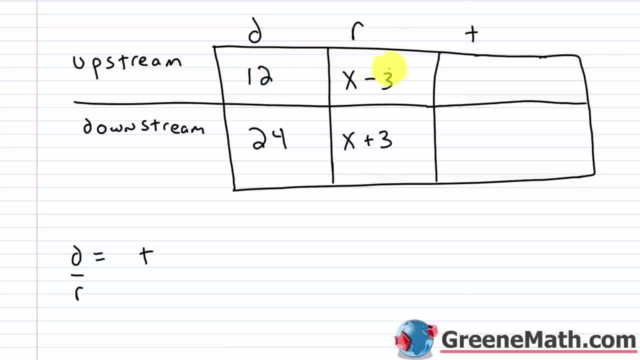 I have a distance here, I have a rate here, So I'm going to have a time. The distance in this case is 12.. The rate in this case Is x minus 3.. So my time For going upstream is 12.. 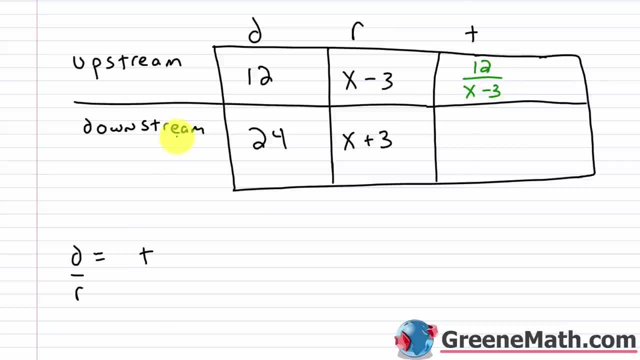 Over x minus 3.. And for downstream, I can do the same exact thing. My time is going to be 24., Which is my distance Over x plus 3., Which is my rate, Now that we have all this information figured out. 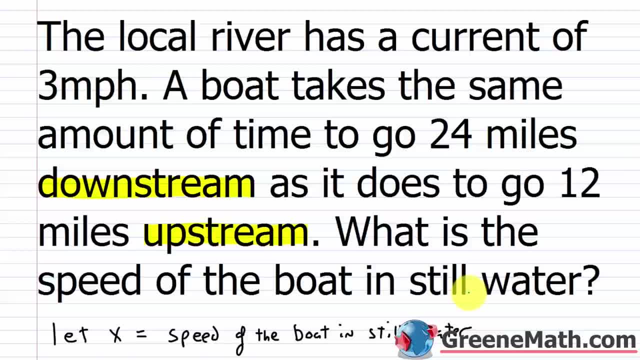 We want to go ahead and set up an equation And, as I told you, When we look at this problem, It tells us that a boat takes the same amount of time, The same amount of time, To go 24 miles downstream As it does to go 12 miles upstream. 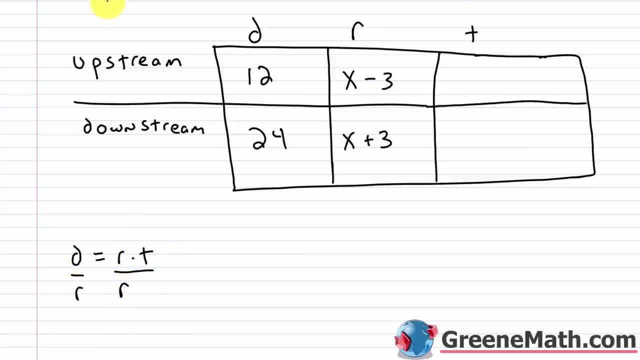 so I divide both sides of the equation by r to isolate t as we did earlier this cancels with this and I've got t by itself so time is equal to distance over rate I have a distance here I have a rate here so I'm going to have a time the distance in this case is 12 the rate in this case is x minus 3 so my time for going upstream is 12 over x minus 3 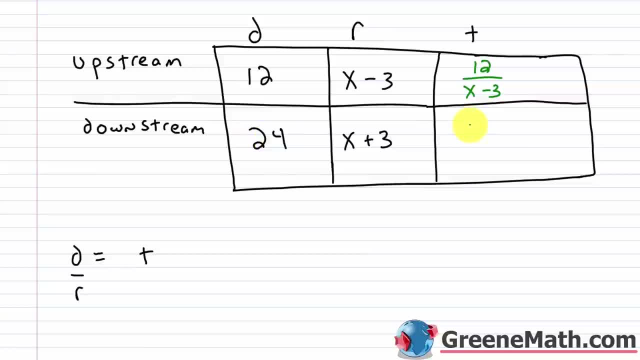 and I can do the same exact thing my time is going to be 24 which is my distance 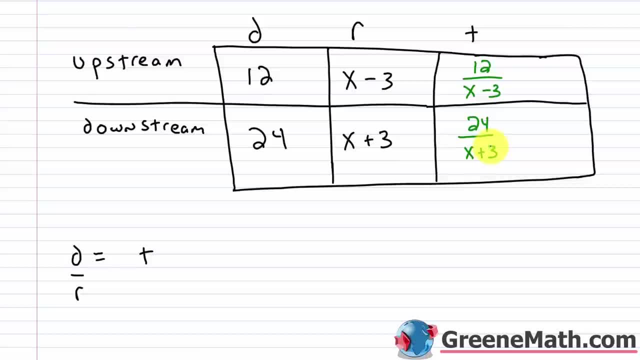 over x plus 3 which is my rate now that we have all this information figured out we want to go ahead and set up an equation 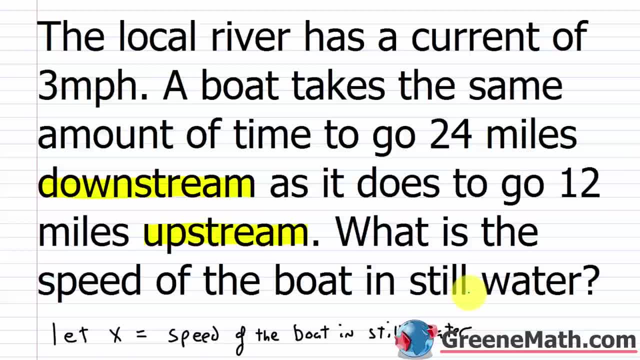 and as I told you when we look at this problem it tells us that a boat takes the same amount of time the same amount of time 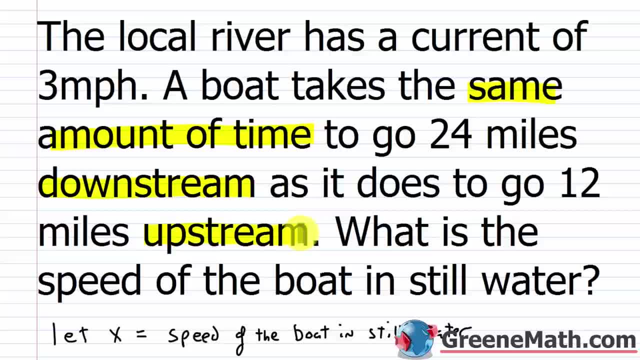 to go 24 miles downstream as it does to go 12 miles upstream so that means I can set the two times equal 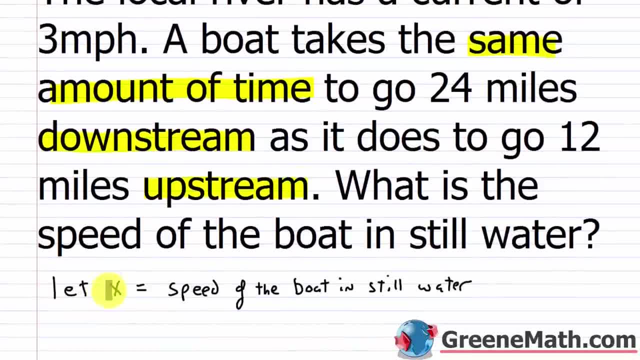 to each other and I could solve for x and I'd figure out what the speed of the boat is in still water 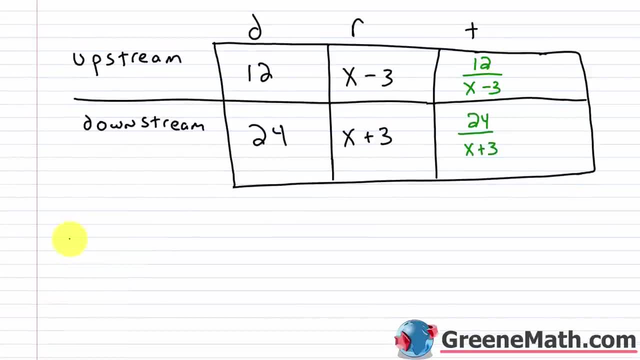 let me erase this real quick so I have the time for upstream 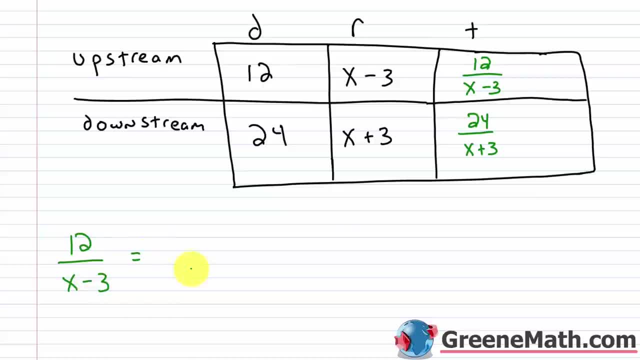 which is 12 over x minus 3 and I'm going to set this equal to the time for downstream which is 24 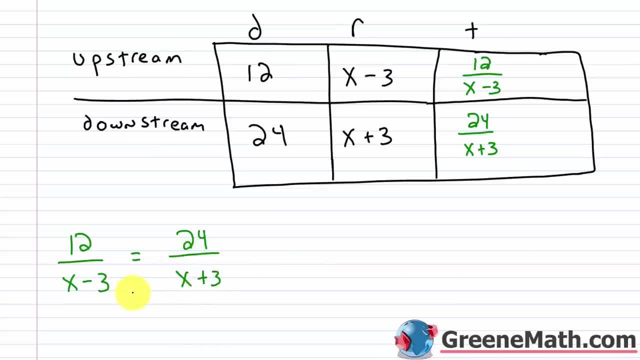 over x plus 3 so in the last section we learned how to solve equations of this form so one way we can do this is we can find the LCD 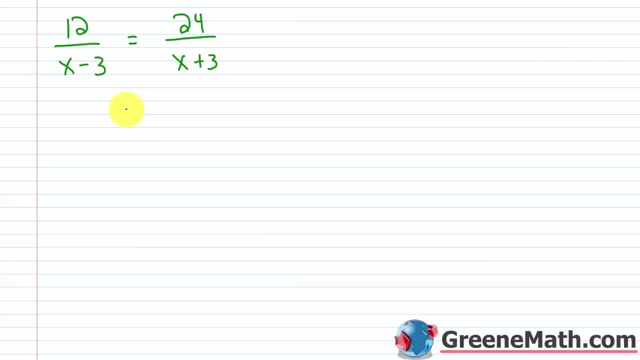 and multiply both sides of the equation by the LCD clear the equation of any denominators and kind of go from there but in this particular scenario the easiest thing to do would be to cross multiply remember that from proportions I can multiply x minus 3 that quantity times 24 and I can multiply x plus 3 that quantity times 12 and why is that a shortcut well the LCD here is going to be what it's x minus 3 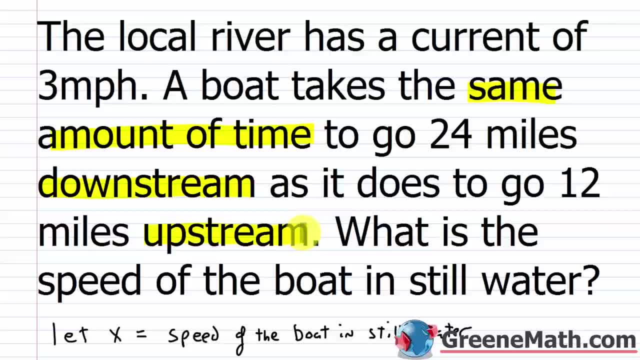 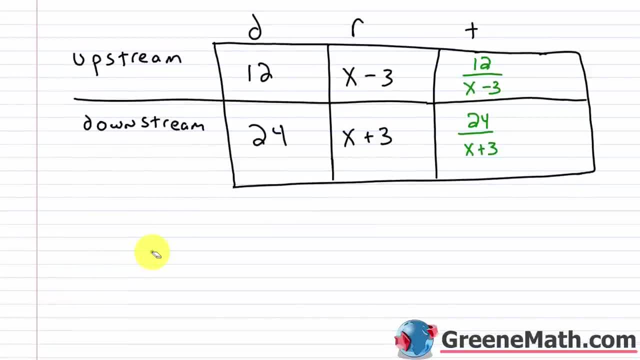 So that means I can set the two times equal to each other And I can solve for x And I can figure out what the speed of the boat is In still water. Let me erase this real quick, So I have the time for upstream. 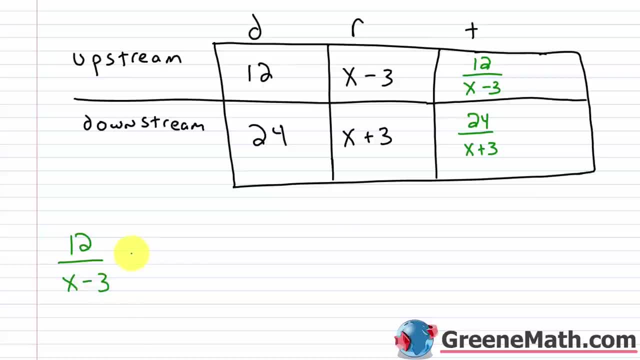 Which is 12 over x minus 3.. And I'm going to set this equal to The time for downstream, Which is 24. Over x plus 3.. So in the last section We learned how to solve Equations of this form. 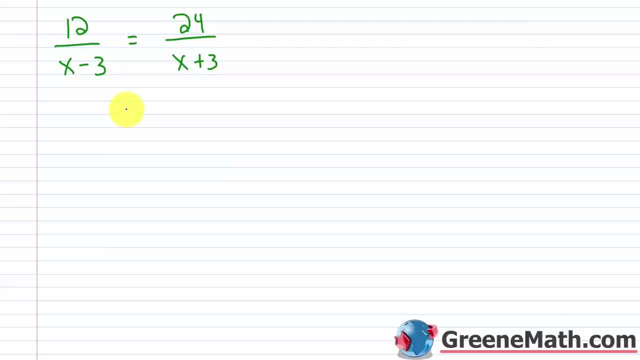 So one way we can do this Is to take the LCD And multiply both sides of the equation By the LCD, Clear the equation of any denominators And kind of go from there. But in this particular scenario The easiest thing to do- 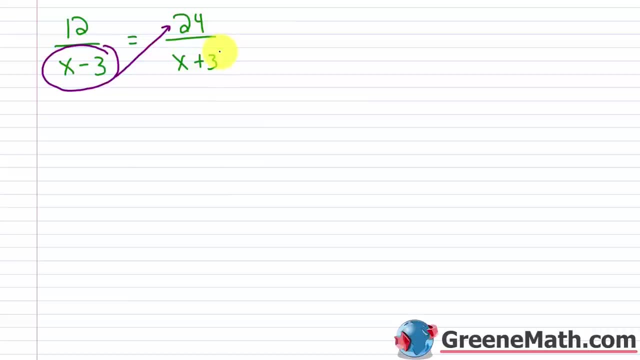 Would be to cross multiply. Remember that from proportions. I can multiply x minus 3.. That quantity times 24.. And I can multiply x plus 3. That quantity times 12.. And why is that a shortcut? Well, the LCD here. 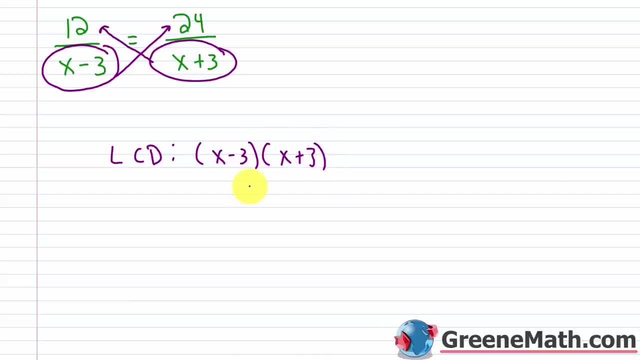 Is going to be x plus 3.. So if I multiply both sides of the equation By this LCD, Well what's going to happen is This denominator here is going to cancel, And I'm going to multiply 24 by x minus 3.. 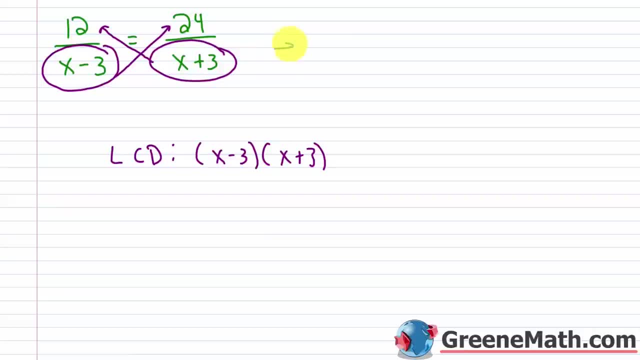 Which is exactly what I'm doing When I'm cross. multiplying This would be 24 times the quantity x minus 3.. Is equal to Same thing over here. The x minus 3 would cancel And I'd be multiplying 12 by x plus 3.. 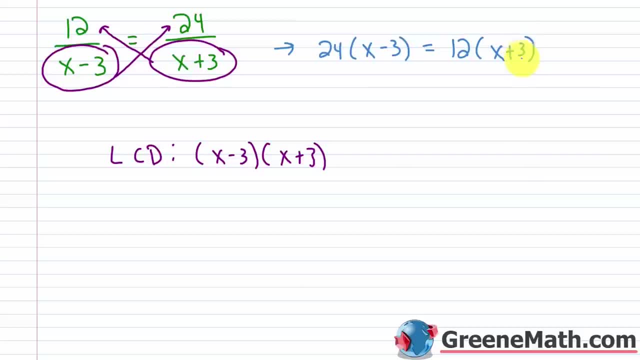 That's what I'm doing when I'm cross multiplying, So that's a little shortcut for you To kind of speed up the process. If you get this scenario, Let's erase this real quick. And so 24 times x Is 24x. 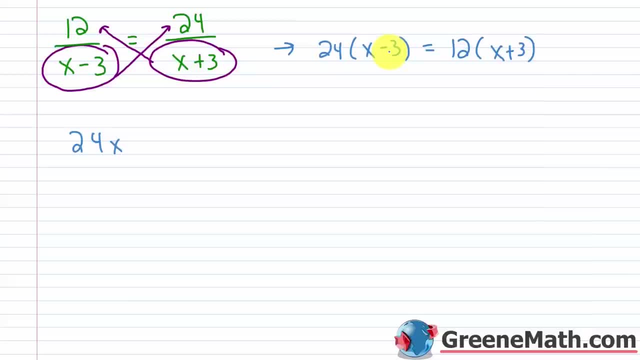 And then 24 times negative 3. Is going to give me negative 72. And this is equal to Over. here we have 12 times x, That's 12x. And then we have 12 times 3. That's 36.. 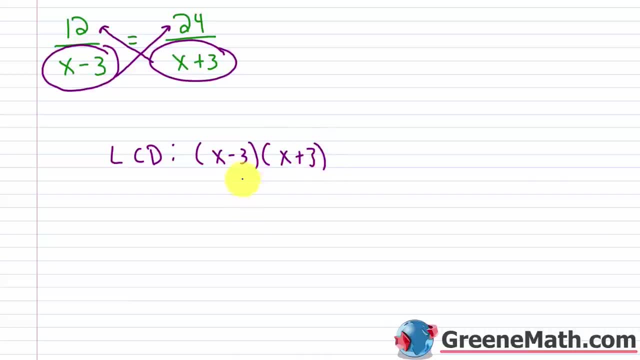 x plus 3 so if I multiply both sides of the equation by this LCD well what's going to happen is this denominator here is going to cancel and I'm going to multiply 24 by x minus 3 which is exactly what I'm doing when I'm cross multiplying this would be 24 times the quantity x minus 3 is equal to same thing over here the x minus 3 would cancel and I'd be multiplying 12 by x plus 3 that's what I'm doing when I'm cross multiplying so 12 times the quantity x plus 3 so that's a little shortcut 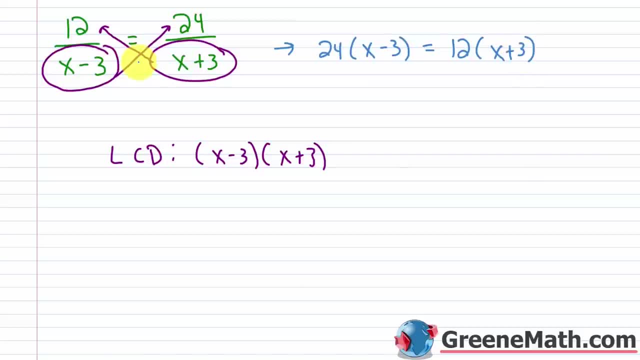 for you to kind of speed up the process if you get this scenario so let's erase this real quick and so 24 times x is 24x and then 24 times negative 3 is going to give me negative 72 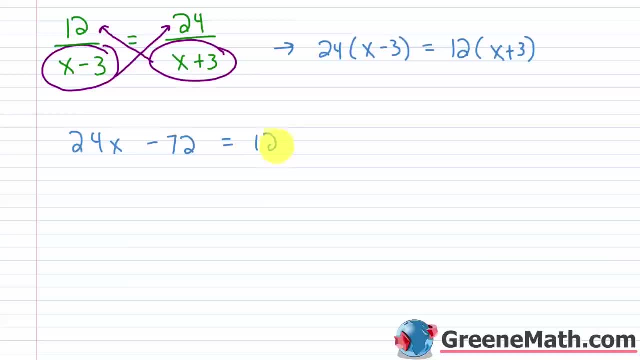 and this is equal to over here we have 12 times x that's 12x and then we have 12 times 3 that's 36 ok so let's solve this equation very very easy to do I'm just going to add 72 to both sides of the equation 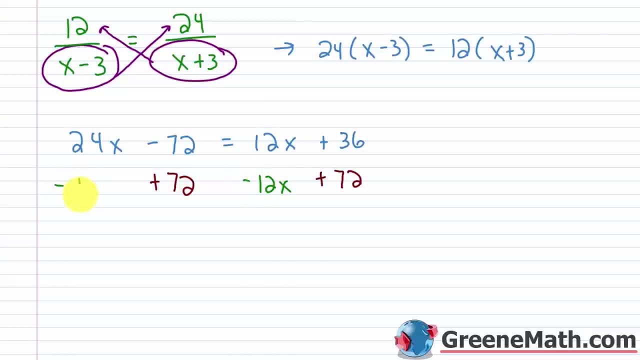 and I'm going to subtract 12x from both sides of the equation so this is going to cancel and this is going to cancel 24x minus 12x is 12x so this is 12x and this is equal to 36 plus 72 which is 108 ok as my last step here I'm going to divide both sides of the equation by 12 and this is going to cancel with this and I'm going to have that x is equal to 9 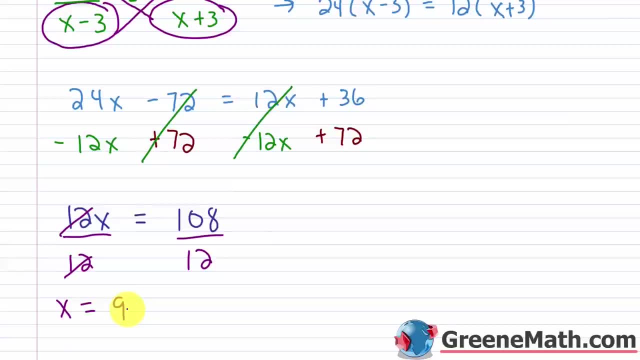 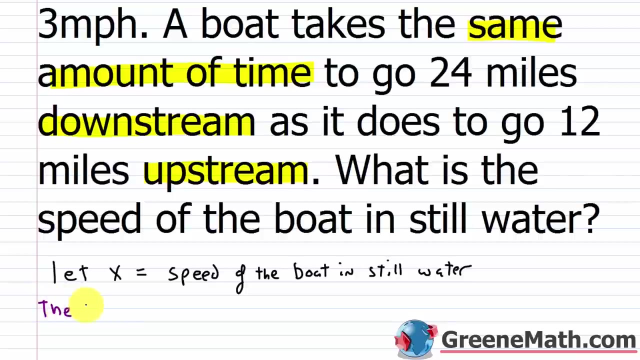 so I found the answer to the problem x again was the speed of the boat in still water and that's what I was trying to figure out so x is equal to 9 so the speed of the boat in still water is 9 miles per hour so let's go back up to the top and write that so I'm just going to write that the boat travels 9 miles per hour in still water and that answers our question there what is the speed of the boat in still water so how would we check something like this well let's read back through the problem real quick 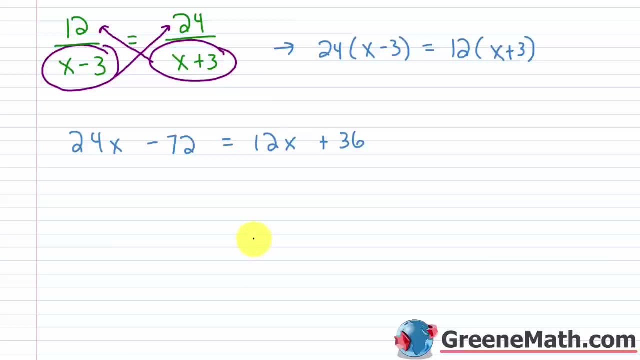 Okay, so let's solve this equation. Very, very easy to do. I'm just going to add 72. To both sides of the equation And I'm going to subtract 12x from both sides of the equation. So this is going to cancel. 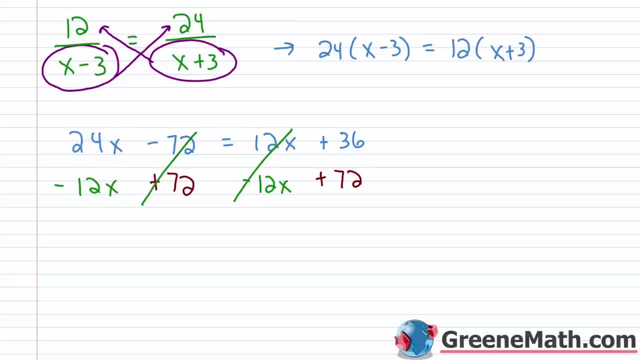 And this is going to cancel. 24x minus 12x is 12x, So this is 12x, And this is equal to 36 plus 72.. Which is 108.. Okay, as my last step here, I'm going to divide both sides of the equation by 12.. 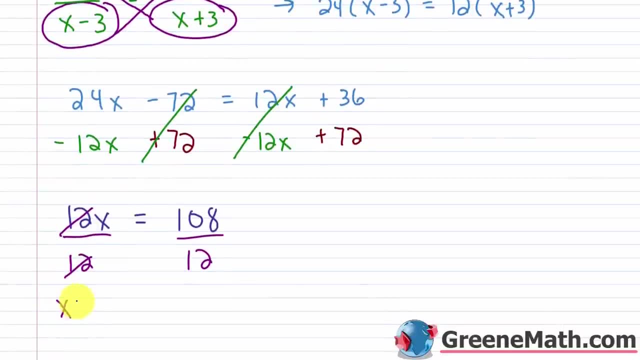 And this is going to cancel with this And I'm going to have that x is equal to 9.. So I've found the answer to the problem. x again was the speed of the boat In still water, And that's what I was trying to figure out. 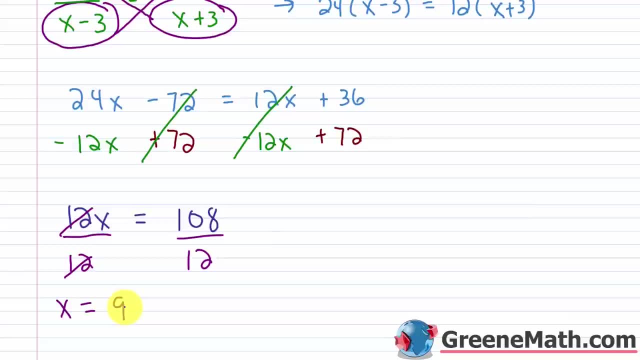 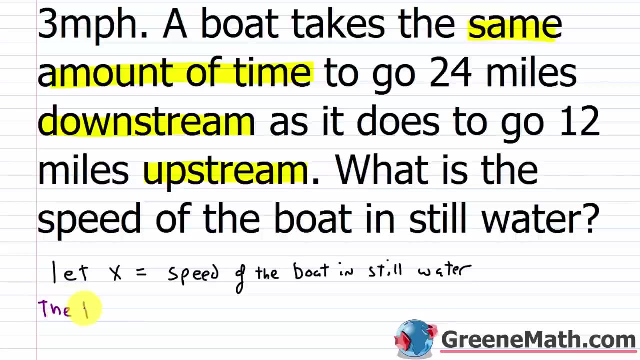 So x is equal to 9.. So the speed of the boat in still water Is 9 miles per hour. So let's go back up to the top and write that. So I'm just going to write that the boat Travels. 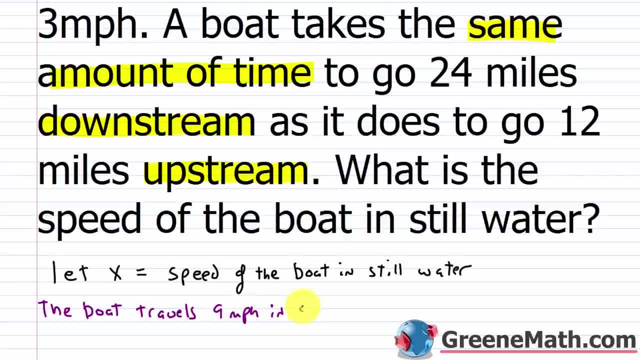 9 miles per hour In still water, In still water- And that answers our question there- What is the speed of the boat in still water? So how would we check something like this? Well, let's read back through the problem real quick. 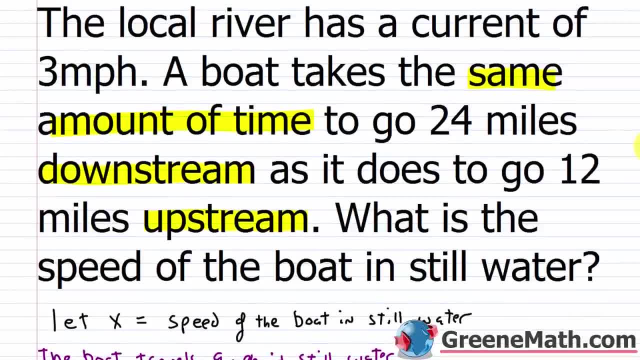 So the local river has a current of 3 miles per hour. A boat takes the same amount of time to go 24 miles downstream Again with the current As it does to go 12 miles upstream Again against the current. 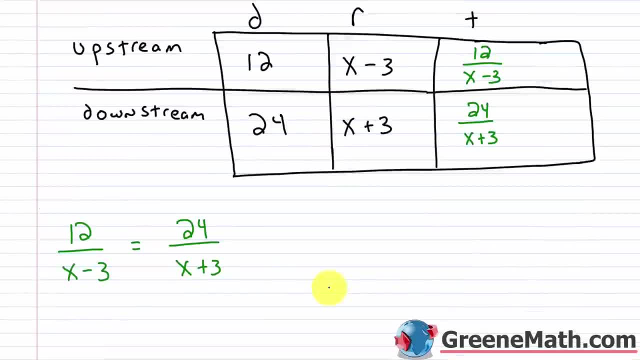 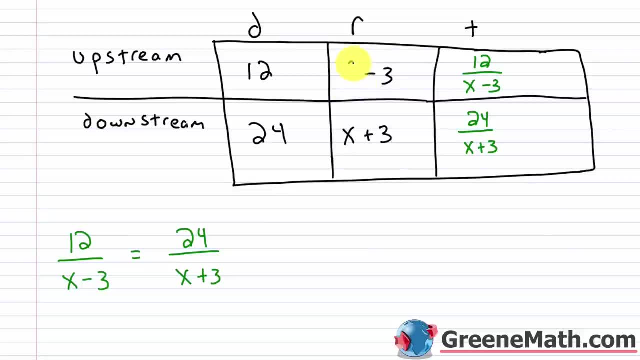 So what is the speed of the boat in still water? So I know at this point that Upstream Is going to be what? Well, x is 9.. So I plug in a 9 there. 9 minus 3 is 6.. 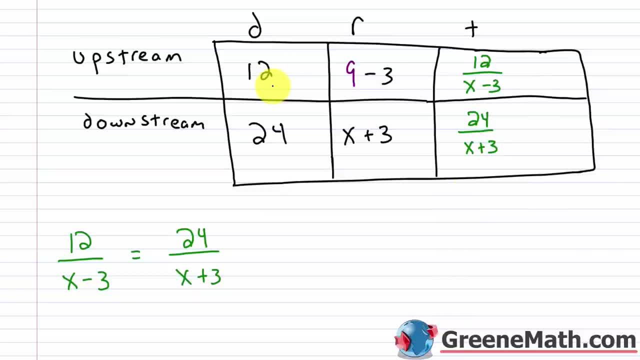 So, in other words, I know that the time that it takes to go 12 miles Upstream Should be 12 over 9 minus 3.. Or 12 over 6, which is 2.. And is that equal to The amount of time that it takes to go downstream? 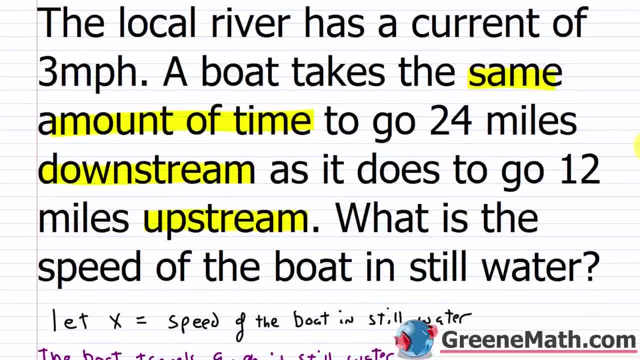 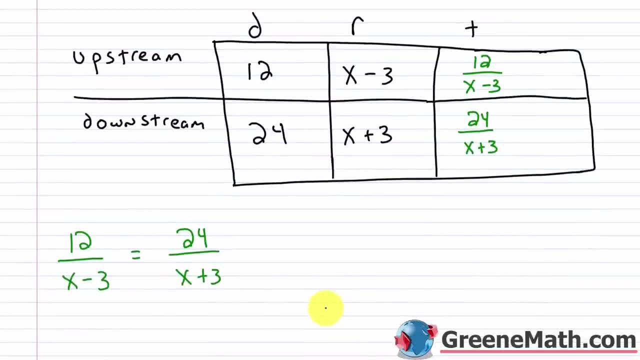 so the local river has a current of 3 miles per hour a boat takes the same amount of time to go 24 miles downstream again with the current as it does to go 12 miles upstream again against the current so what is the speed of the boat in still water so I know at this point that upstream my rate of speed is going to be what well x is 9 so I plug in a 9 there 9 minus 3 is 6 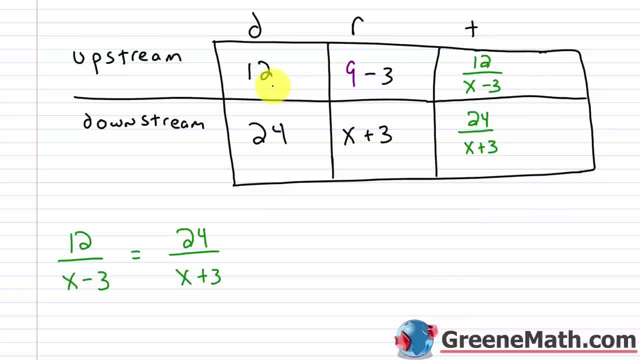 so in other words I know that the time that it takes to go 12 miles upstream should be 12 over 9 minus 3 or 12 over 6 which is 2 and is that equal to the amount of time that it takes to go downstream well my speed downstream if I replace this x with a 9 9 plus 3 is 12 is 12 miles per hour you basically have 24 over 12 so 24 over 12 would be 2 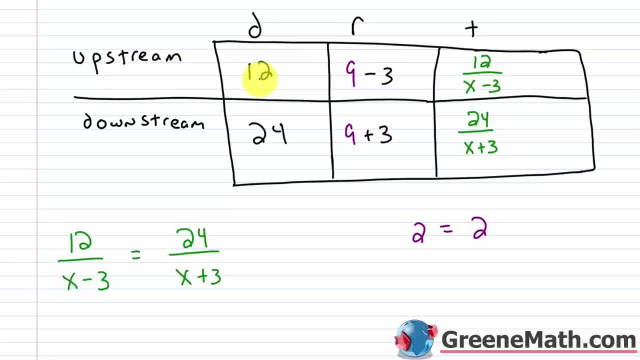 so it takes the same amount of time which is 2 hours to go upstream 12 miles as it does to go downstream 24 miles 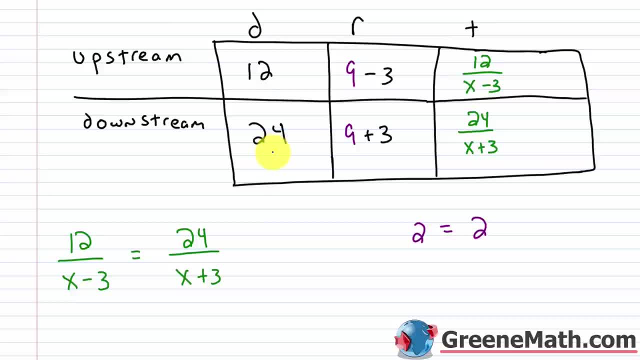 so we have the correct answer here the speed of the boat in still water is 9 miles per hour 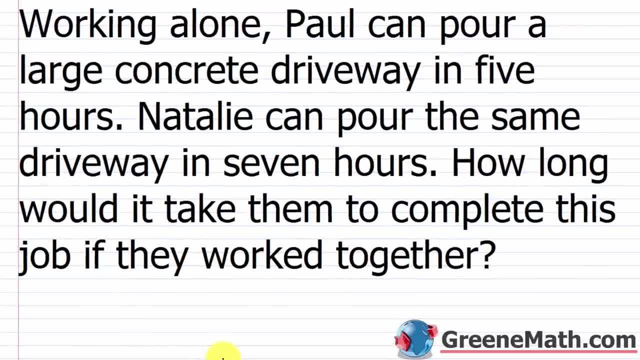 so the next type of problem we are going to deal with is known as a work rate problem or some of you will hear it called a rate of work problem either way these types of problems involve how much time it takes to complete a job so in this scenario 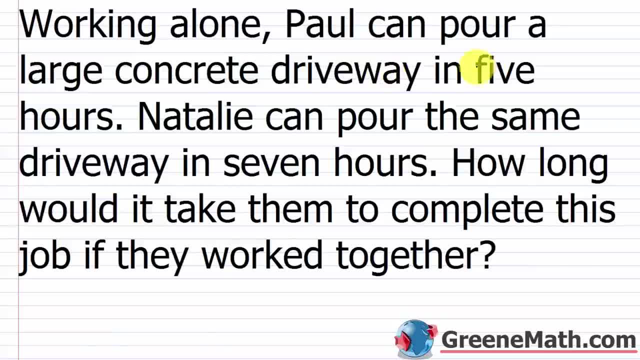 working alone Paul can pour a large concrete driveway in 5 hours 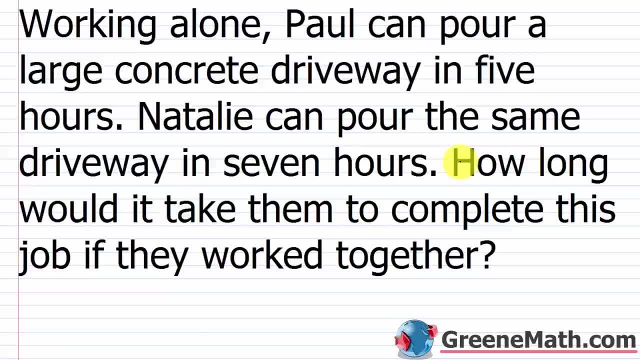 Natalie can pour the same driveway in 7 hours 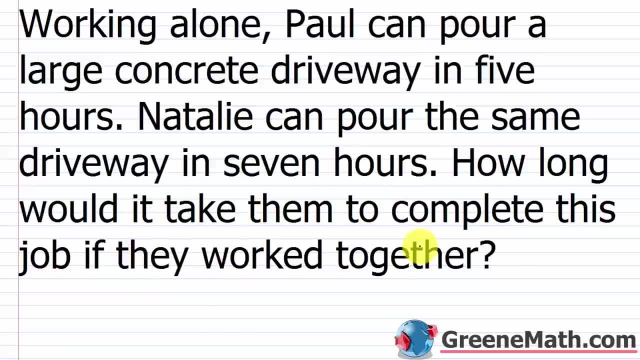 how long would it take to complete this job if they worked together 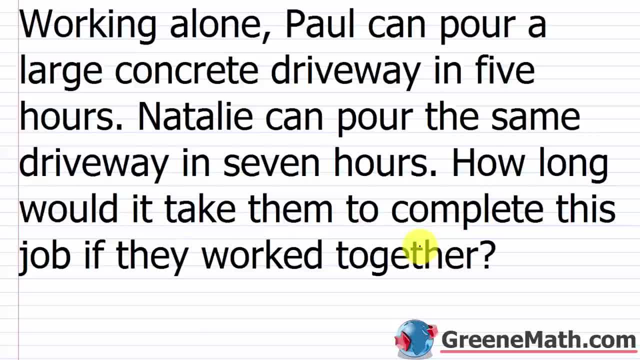 so when you first start thinking about it if you don't get any direction on it it's kind of hard to figure out how to solve this 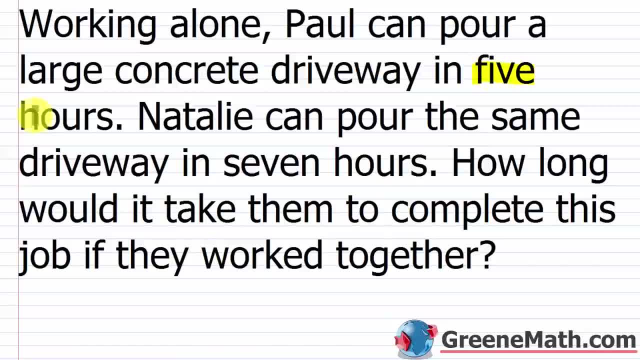 I know how long it would take for Paul to pour a driveway it's 5 hours I know how long it would take for Natalie to pour the same driveway 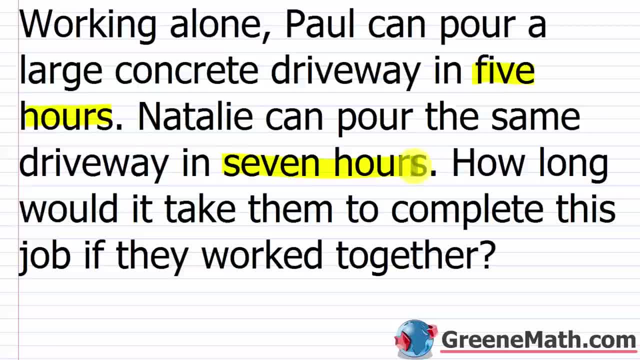 it's 7 hours but if I combine their work rates and they work together how long is it going to take 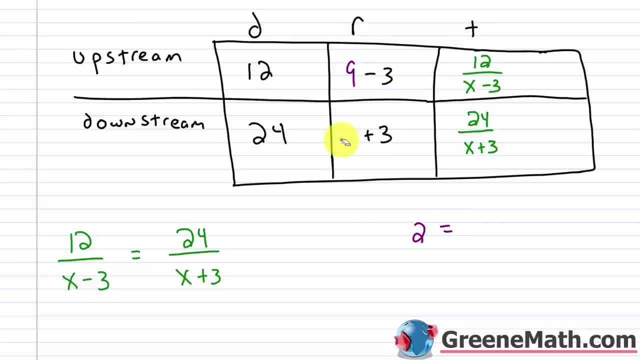 Well, my speed downstream, If I replace this x with a 9. 9 plus 3 is 12. Is 12 miles per hour. So I basically have 24 over. Again. 9 plus 3 is 12.. So 24 over 12 would be 2.. 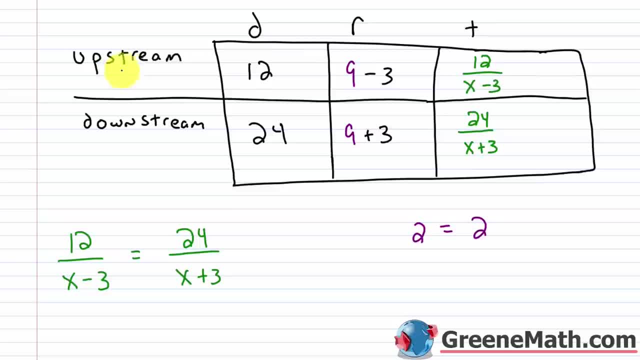 So it takes the same amount of time, Which is 2 hours, To go upstream 12 miles As it does to go downstream 24 miles. So we have the correct answer here. Right, the speed of the boat in still water Is 9 miles per hour. 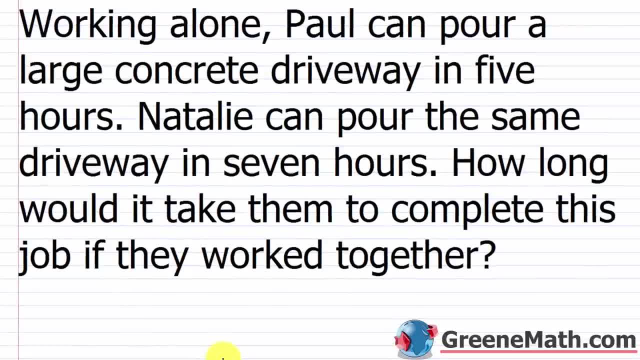 So the next type of problem we are going to deal with Is known as a work rate problem, Or some of you will hear it called A rate of work problem. Either way, these type of problems Are not going to be solved By the time you get to the point. 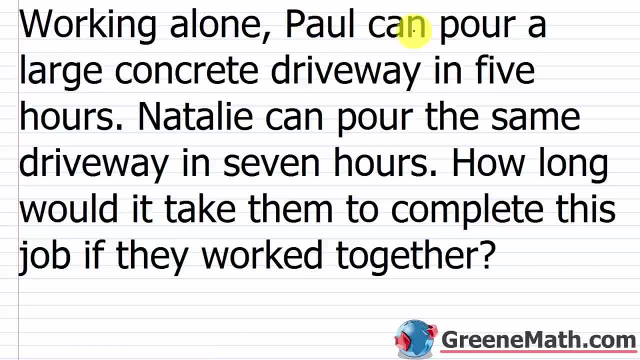 Where you are going to be able to Complete a job. So in this scenario, Working alone, Paul can pour a large concrete driveway In 5 hours. Natalie can pour the same driveway In 7 hours. How long would it take to complete this job? 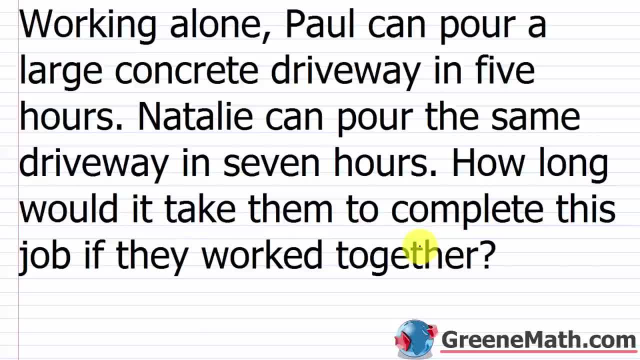 If they worked together. So when you first start thinking about it, If you don't get any direction on it, How long it would take for Paul to pour a driveway- It's 5 hours, It says it right there. I know how long it would take for Natalie to pour the same driveway. 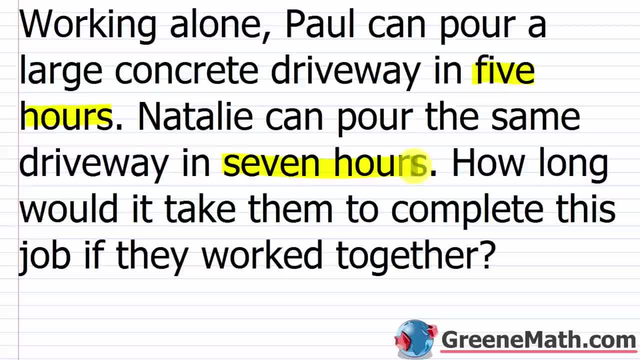 It's 7 hours, But if I combine their work rates And they work together, How long is it going to take? Well, the first thing I have to do is break this down into one unit of time. In this particular case, We are talking about hours. 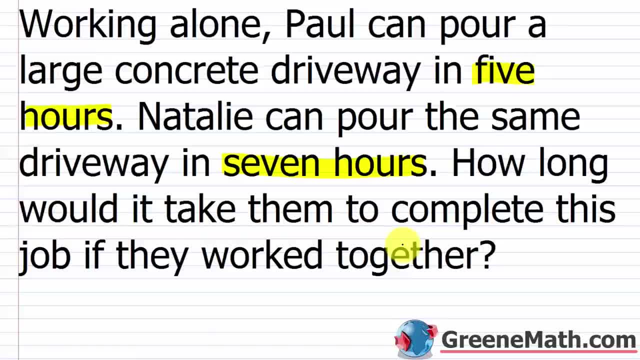 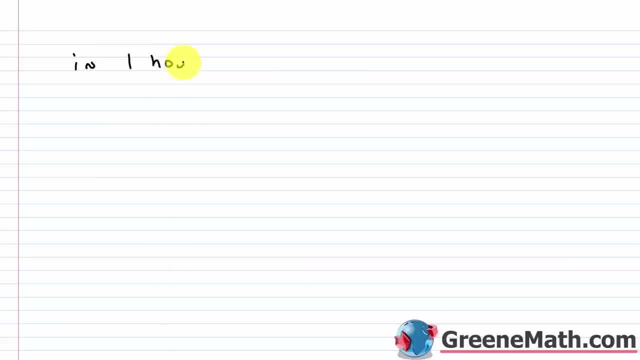 Now for these problems. You might talk about days or weeks or minutes, Whatever it is In one hour, Because I want one unit of whatever time I am dealing with. I am dealing with hours, So I want one of those. What can Paul do in one hour? 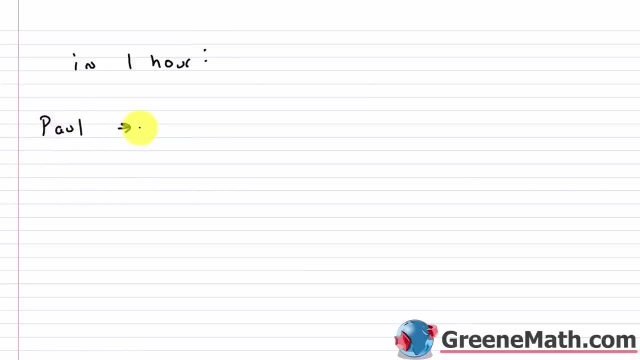 Well, Paul completes the job in 5 hours, So in one hour He has done 1 fifth of the job, 1 fifth of, You could say, the driveway, Or of just the job, Just to be generic, Then, Natalie, 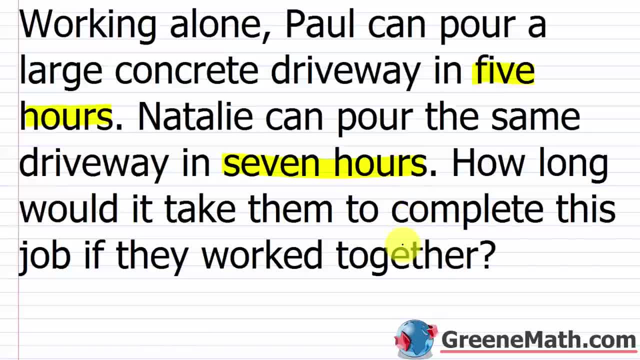 well the first thing I have to do is break this down into one unit of time in this particular case we are talking about hours now for these problems you might talk about days or weeks or minutes whatever it is you are going to break it down 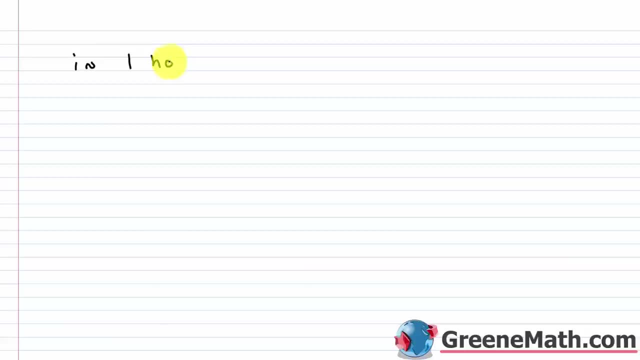 into one of those units of time ok in one hour because I want one unit of water whatever time I am dealing with I am dealing with hours so I want one of those 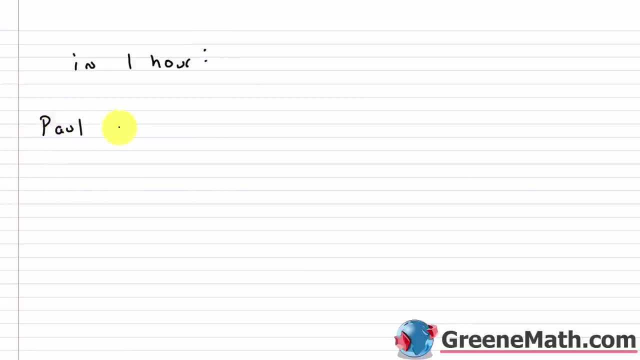 what can Paul do in one hour well Paul completes the job in 5 hours so in one hour he has done one fifth of the job one fifth of 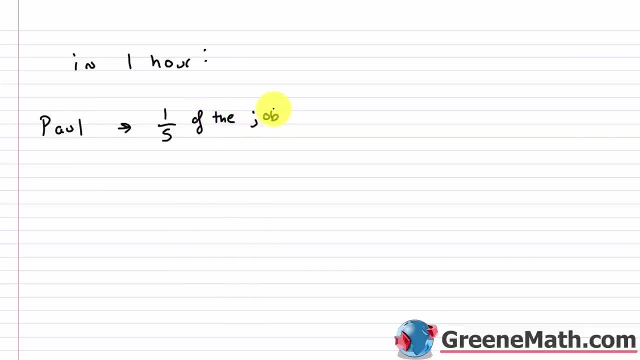 you could say the driveway or of just the job just to be generic then Natalie 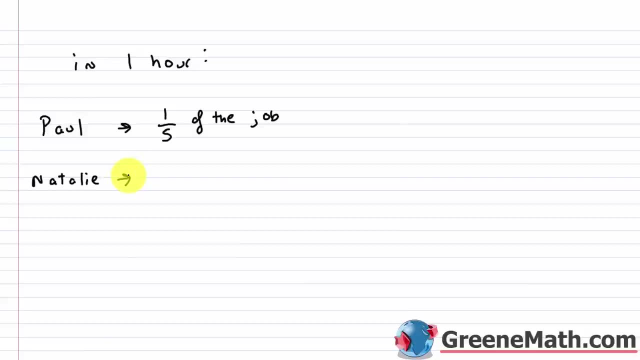 she is a little bit slower she has 7 hours to complete the job so in one hour she is one seventh complete so one seventh of the job 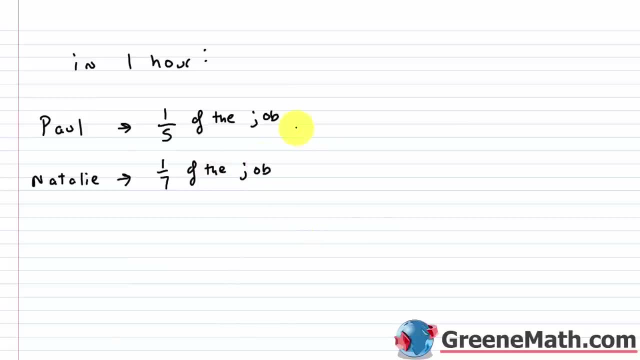 or again you could say of the driveway so what I want to do next is sum the individual contributions from these two people if I do that I am going to get the amount of the job that is completed by both of them in a one hour period again working together so what I want to do here is do one fifth that's the contribution from Paul plus one seventh that's the contribution from Natalie so I would get a common denominator here this would be times 5 over 5 this would be times 7 over 7 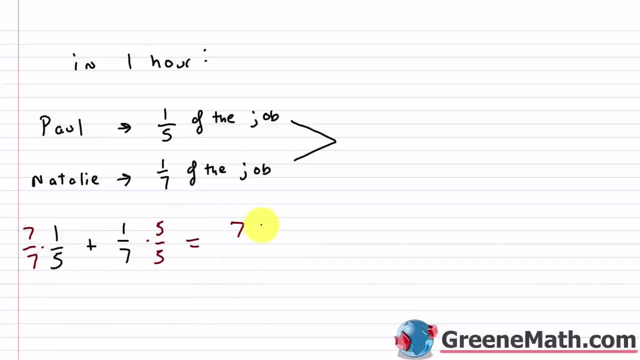 and this would be what 7 plus 5 over 7 times 5 is 35 so 7 plus 5 is 12 so this would be 12 over 35 and what 12 over 35 is that's the contribution again by both of them in a one hour period let me just scroll this down here and say 12 over 35 of the job completed 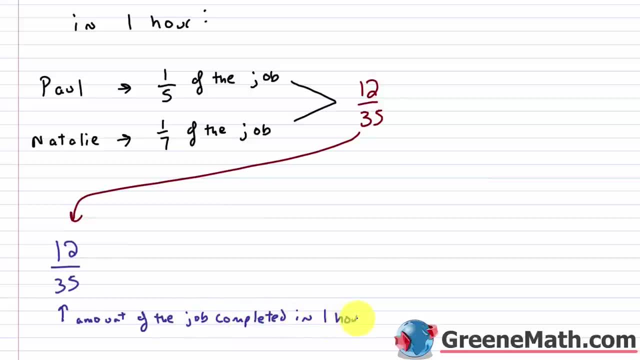 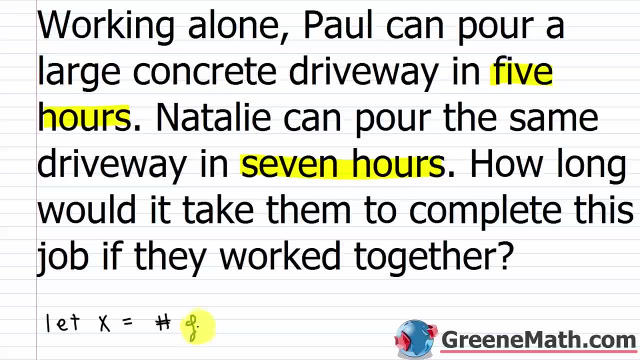 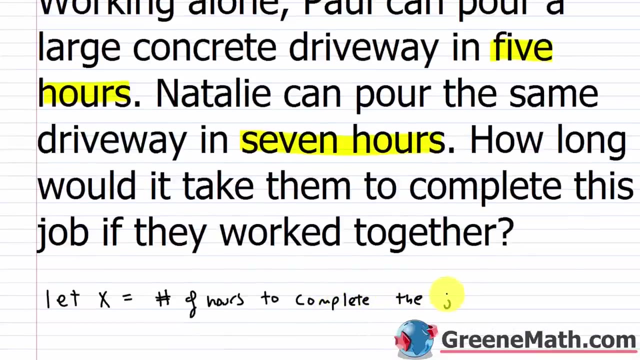 in one hour I am going to let x here be equal to the number of hours to complete the job in if they work together 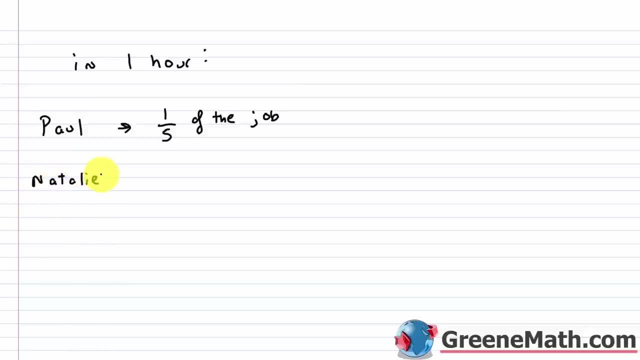 She is a little bit slower. It takes her 7 hours to complete the job, So in one hour She is 1 seventh complete, So 1 seventh of the job, Or again you could say of the driveway. So what I want to do next. 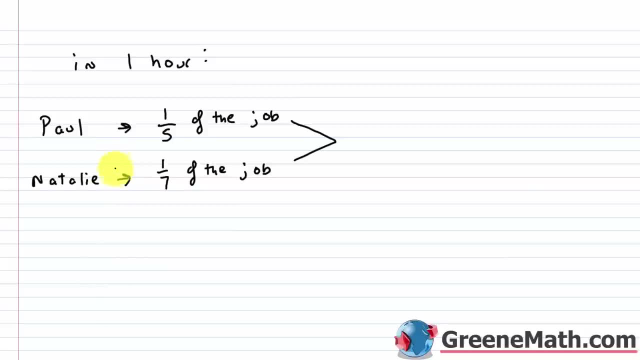 Is sum the individual contributions From these two people. If I do that, I am going to get the amount of the job that is completed By both of them In a one hour period. So what I want to do here Is do 1. fifth, 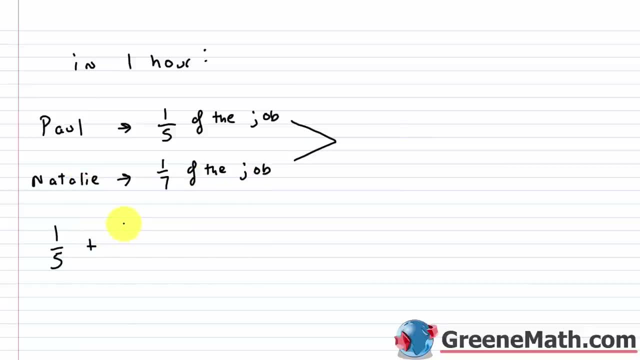 That is the contribution from Paul, Plus 1 seventh, That is the contribution from Natalie. So I would get a common denominator here. This would be times 5 over 5.. This would be times 7 over 7. And this would be what. 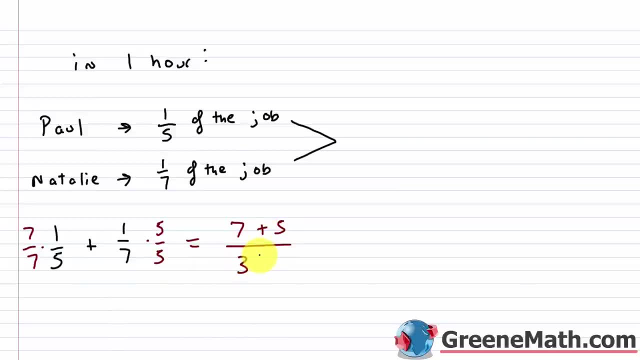 7 plus 5 over 7 times 5 is 35. So 7 plus 5 is 12.. So this would be 12. Over 35 here, And what 12 over 35 is Is the contribution. 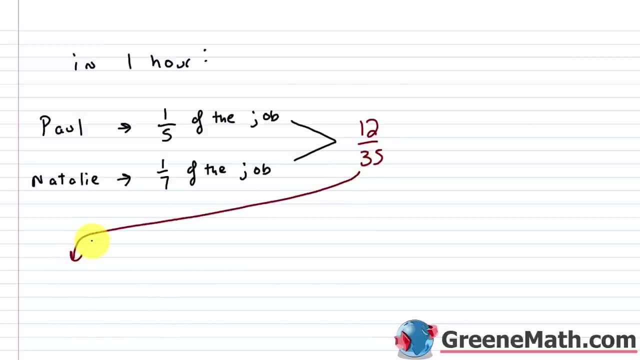 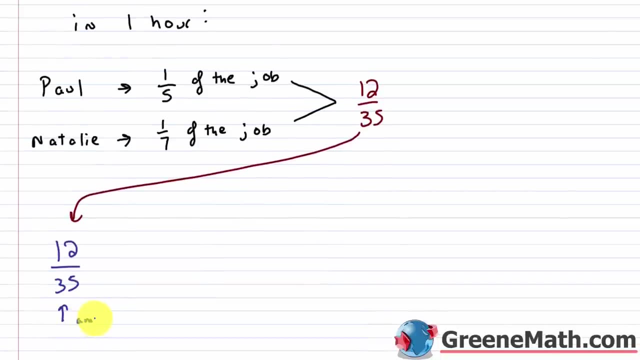 Again, by both of them In a one hour period. So I am just going to scroll this down here And just say 12: thirty fifths Is the amount Of the job Completed In one hour. I am going to. 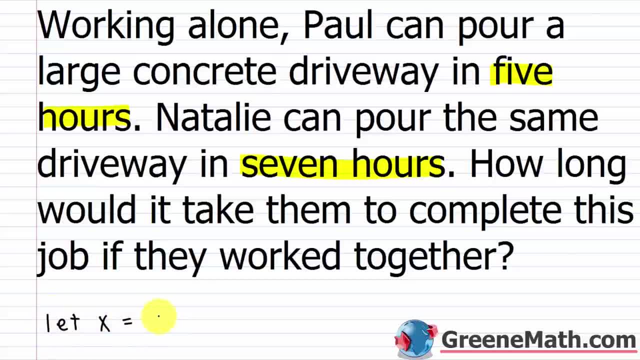 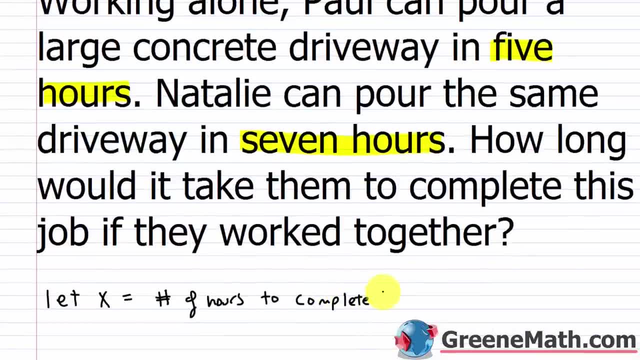 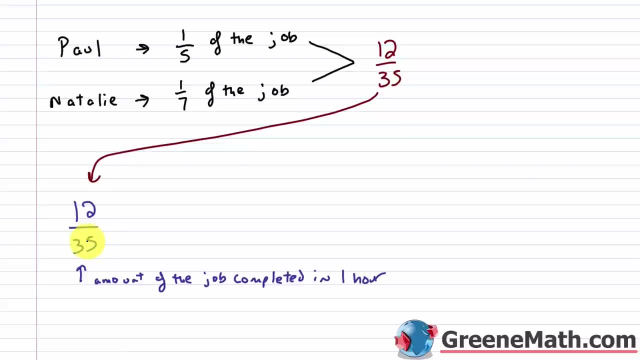 Let x here Be equal to The number of hours To complete The job. If They work together, We have 12 over 35 or 12 thirty fifths Is the amount of the job completed in one hour. 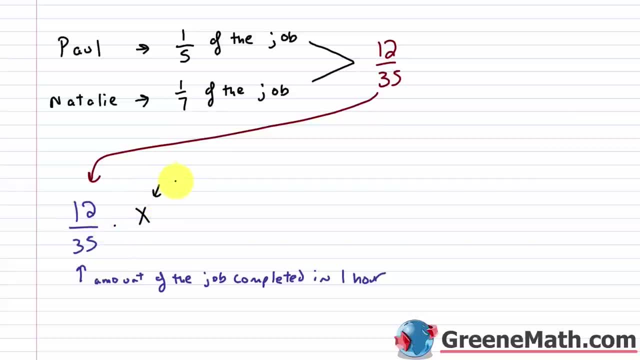 If I multiply this by x, Which is the number of hours, The again number Of hours To complete The job, I am going to get One. Okay, And the reason we use one Is it is one completed job. 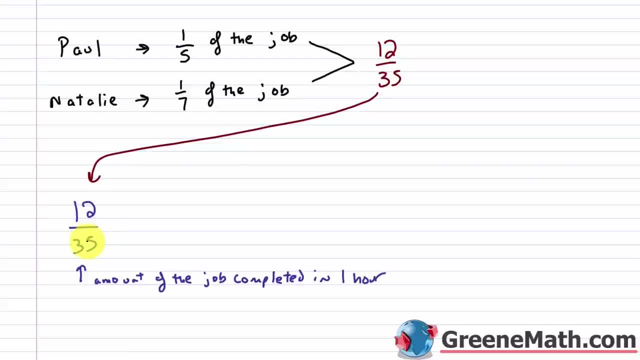 we have 12 over 35 or 12 thirty fifths is the amount of the job completed in one hour if I multiply this by x 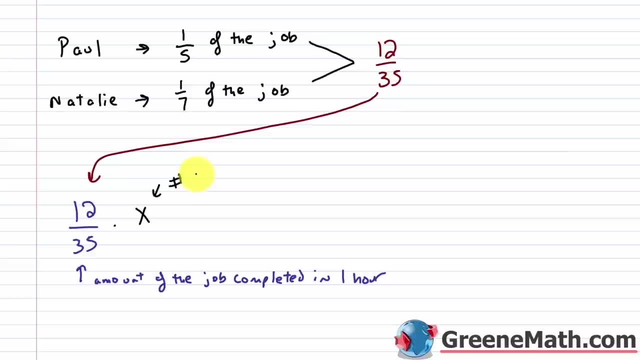 which is the number of hours the again number of hours to complete the job 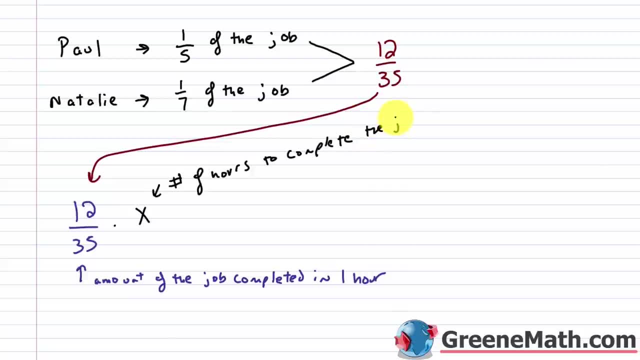 I'm going to get one and the reason we use one is it's one completed job now to make this make sense for you 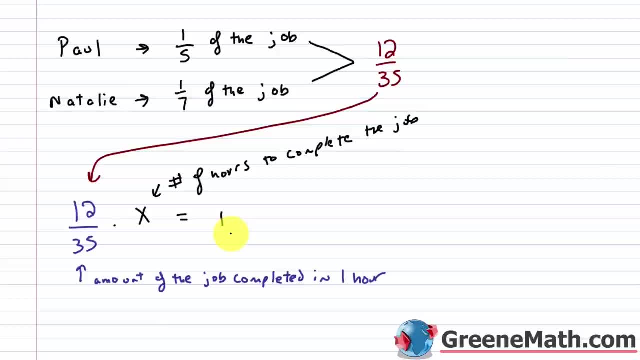 because I know when you start dealing with this it's like why would you set it equal to one 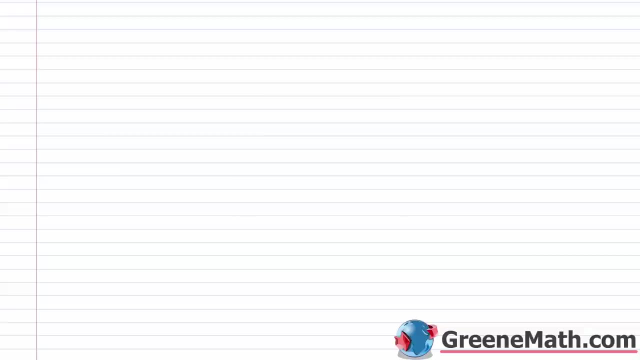 so on and so forth let me just scroll down real quick 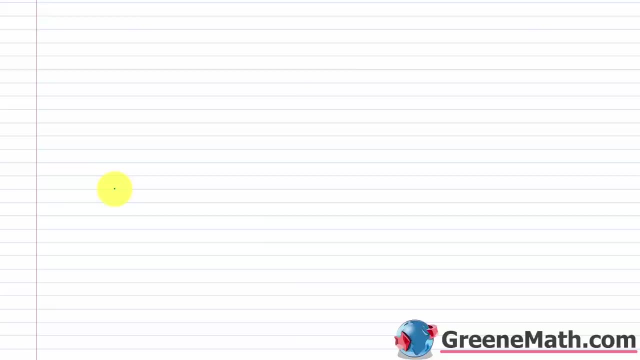 and give you a very easy scenario let's say me and you paint a room in four hours 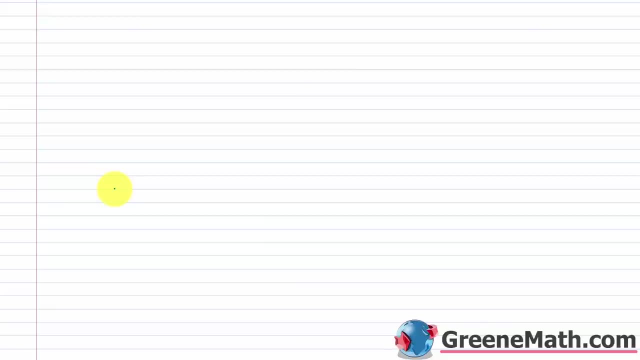 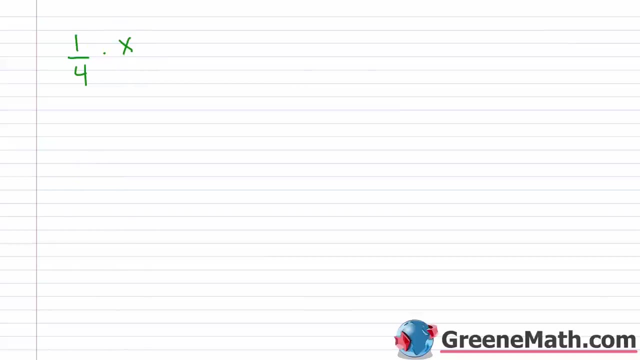 working together so in one hour we would paint a fourth of the room if I didn't know how many hours it would take let's say I multiplied that by x and then I filled in that with a four well I know that four times one fourth is equal to one it's because we're completing one room or one job however you want to think about that so that's our goal is to set this equal to one because we are trying to see how long it's going to take to complete one 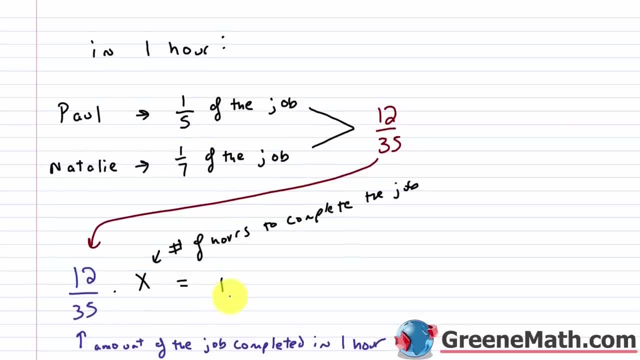 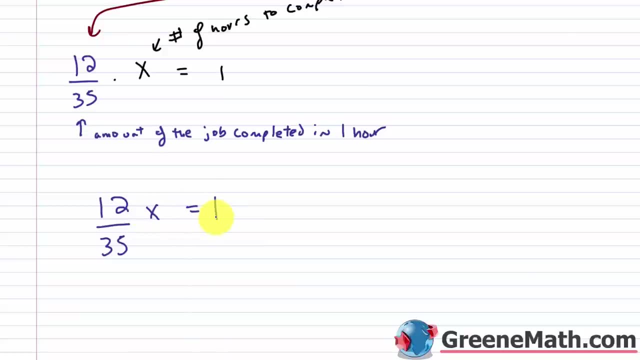 job and now all we need to do is solve this very simple equation if I have twelve thirty fifths x is equal to one all I need to do is multiply both sides by the reciprocal multiply this by thirty five twelfths and this by thirty five twelfths and I'm going to get one this is going to cancel x is equal to thirty five twelfths now let's go back up to the top and make sense of this so I'm just going to answer it first so how long would it take for them to complete this job 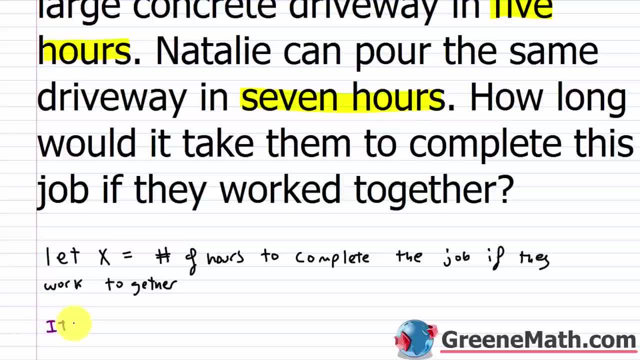 if they worked together it would take 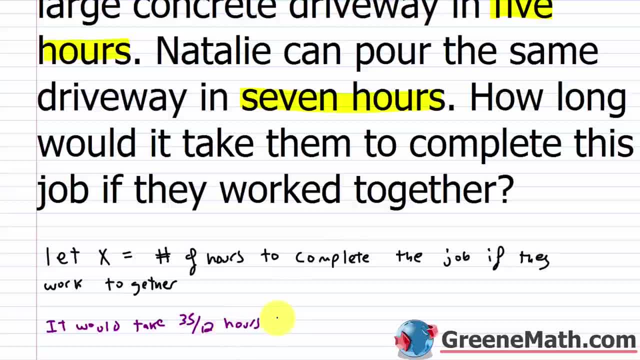 thirty five twelfths hours to complete the job 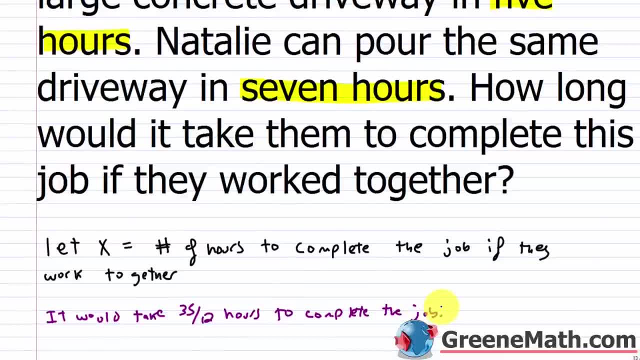 and you can do the division on that it's not going to give you an exact value but it would be two point nine one with a six that repeats forever so you could say about approximately two point nine two hours if you wanted to just give an estimate but if you wanted to be precise 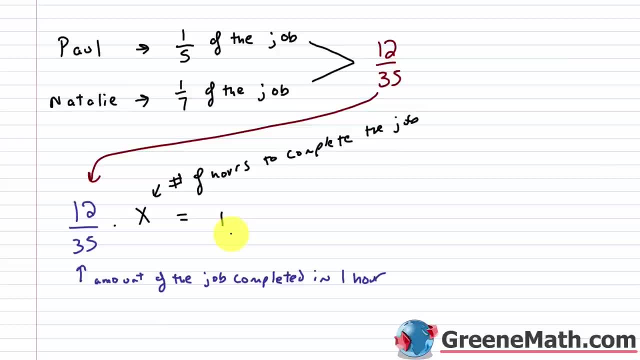 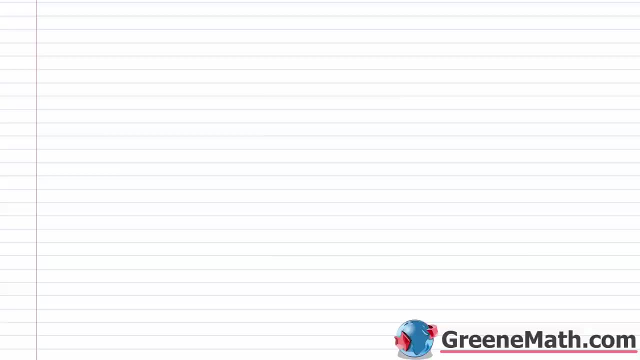 Now To make this make sense for you, Because I know when you start dealing with this, It is like: why would you set it equal to one? So on and so forth. Let me just scroll down real quick And give you a very easy scenario. 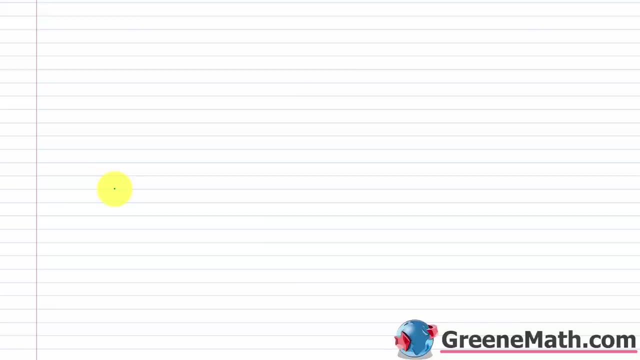 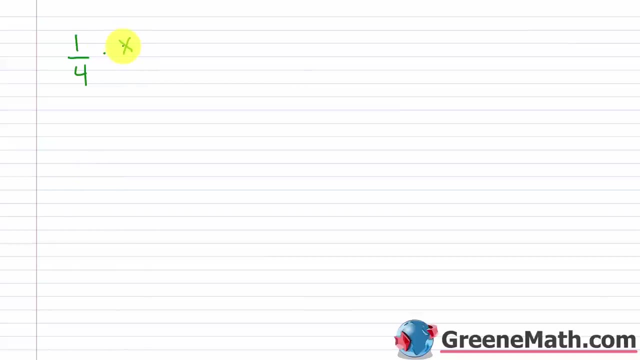 So Let's say We have a room Working together. So that is very, very simple. So in one hour We would paint a fourth of the room. If I didn't know how many hours it would take, Let's say I multiplied that by x. 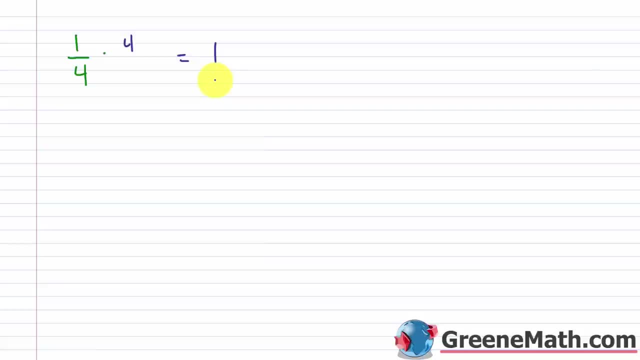 And then I filled in that with a four. Well, I know that Four times one fourth is equal to one. It is because we are completing one room Or one job. So that is how long it is going to take To complete one job. 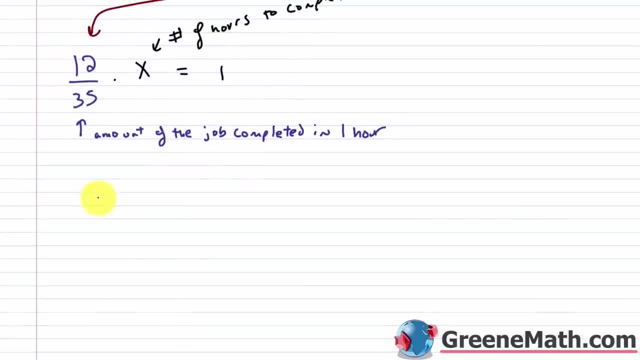 And now all we need to do Is solve this very simple equation: If I have twelve thirty fifths, x Is equal to one. All I need to do is multiply both sides By the reciprocal. Multiply this by thirty five twelfths. 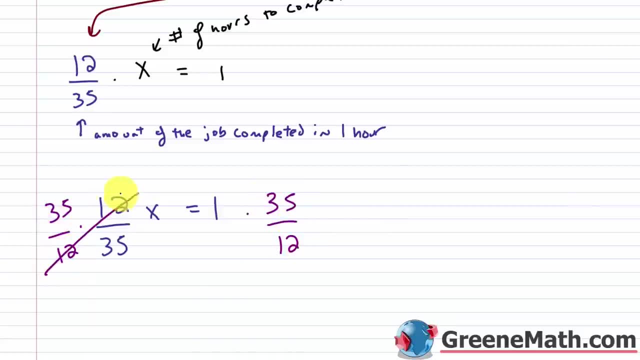 And this by thirty five twelfths, And I am going to get one. This is going to cancel Of. x is equal to thirty five twelfths. Now let's go back up to the top And make sense of this First. 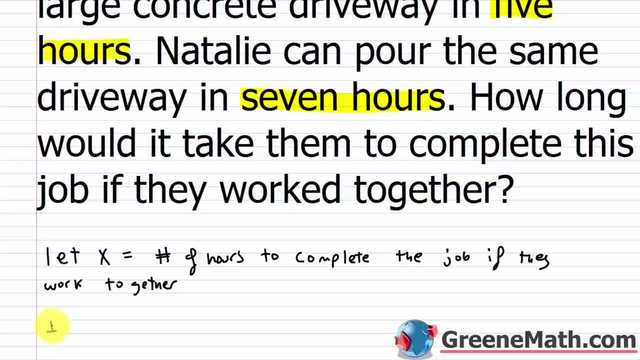 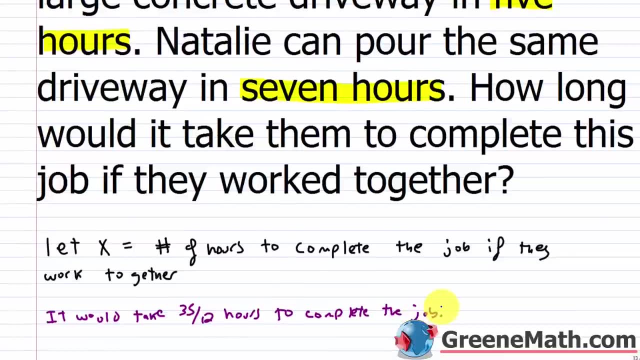 So how long would it take for them to complete this job? If they work together, It would take Thirty five twelfths Hours To complete the job, And you can do the division on that. It is not going to give you an exact value. 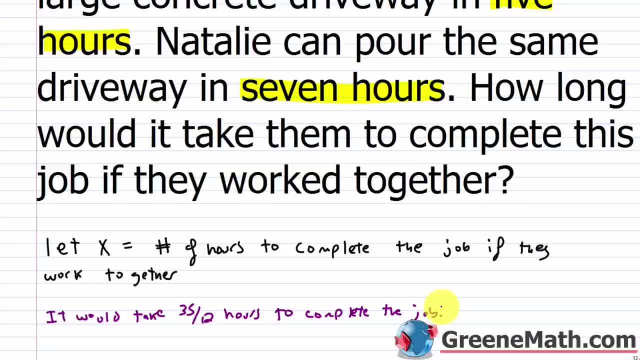 But it would be two point nine, one With a six. that repeats forever. So you could say You know approximately Two point nine, two hours, If you wanted to just give an estimate, But if you wanted to be precise, Which it is good to do on a test. 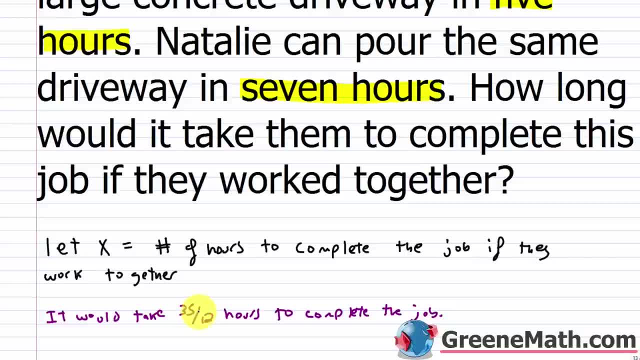 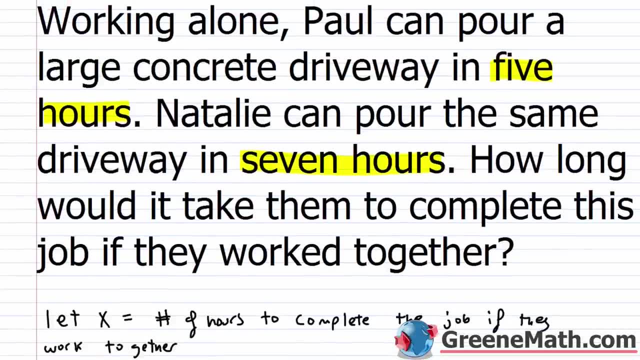 I would just write that fraction that you got, Which is thirty five twelfths Hours. Now, let's make sure that this makes sense. So again, working alone, Paul can pour a large concrete driveway In five hours. Natalie can pour the same driveway in seven hours. 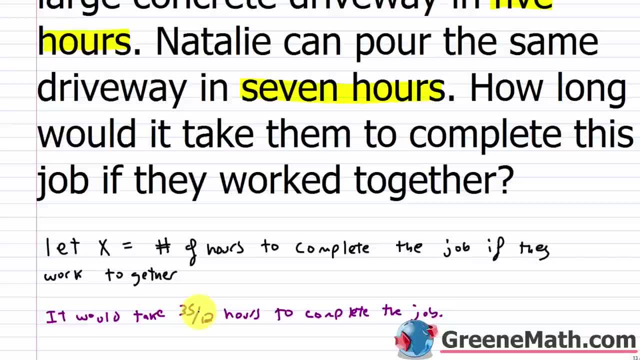 which it's good to do on a test I would just write that fraction that you got 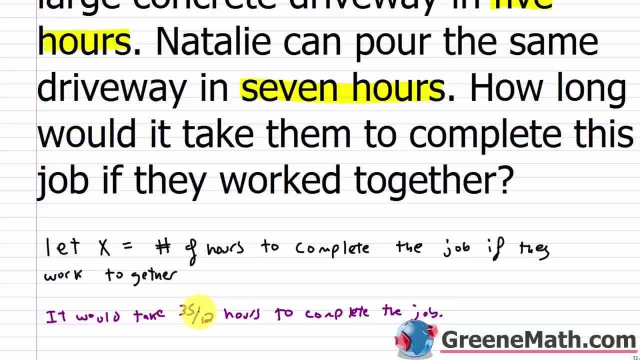 which is thirty five twelfths hours now let's make sure that this makes sense 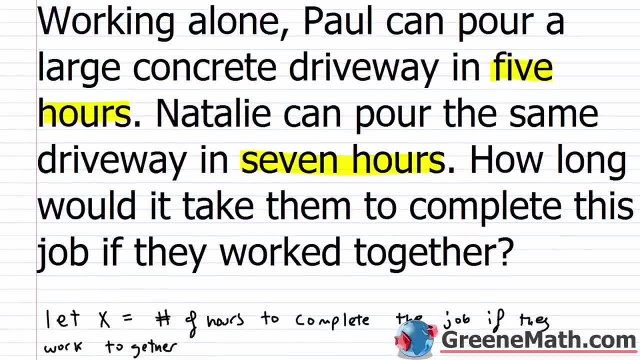 so again working alone Paul can pour a large concrete driveway in five hours Natalie can pour the same driveway in seven hours how long would it take for them to complete this job 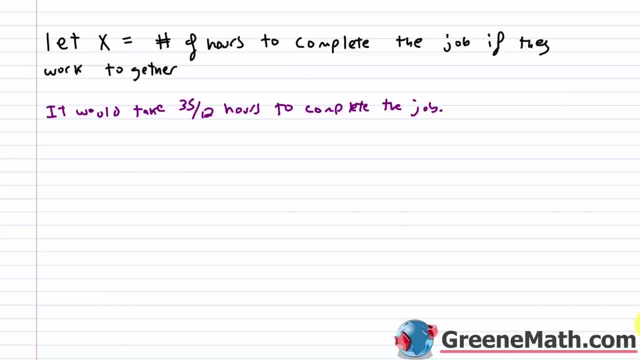 if they worked together so what I'm going to do here is I'm going to take thirty five twelfths which is the number of hours they work for 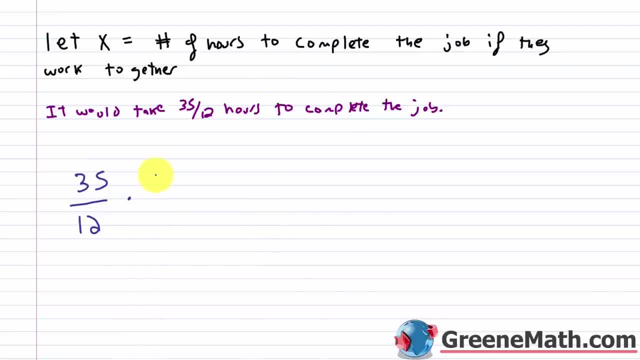 I'm going to multiply this by the rate of speed that Paul works at which is one fifth and then plus I'm going to do thirty five twelfths times the rate of speed that Natalie works at which is one seventh and let's see if this equals one one completed job so this divided by this would give me seven so I'd have seven over twelve so that means that in this amount of time thirty five twelfths hours Paul completes seven twelfths 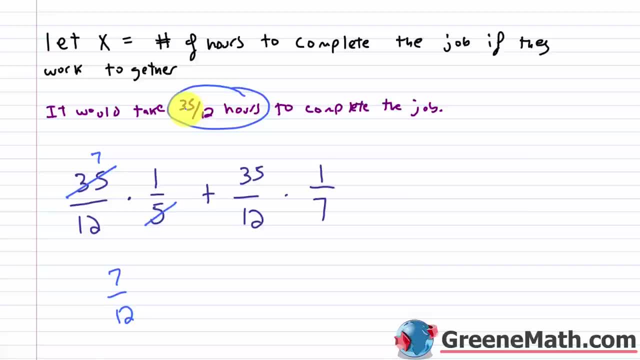 of that driveway he completes seven twelfths of that job you might want to say and then Natalie's contribution is less because she works at a slower rate this divided by this would give me five she does five twelfths of the job so in this amount of time Paul contributes seven twelfths Natalie contributes five twelfths which equals what seven plus five is twelve, twelve over twelve is one one job hello and welcome to algebra one lesson fifty 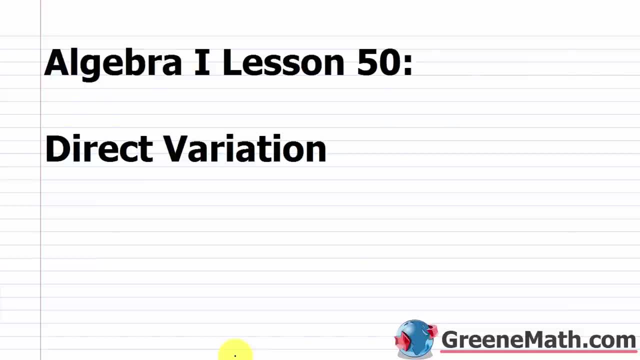 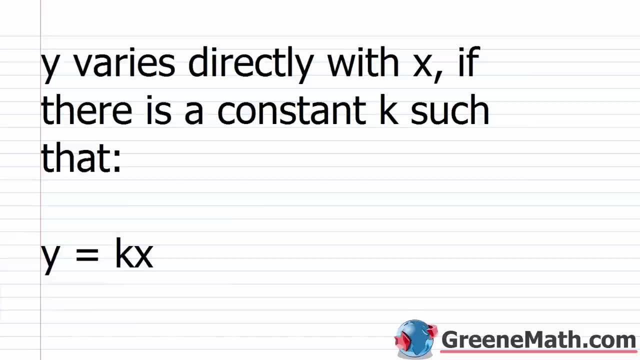 in this video we're going to learn about direct variation so throughout your studies of algebra you're going to encounter many different types of variation obviously as you move higher in algebra you get to algebra two and college algebra you know so on and so forth the types of variation that you're going to encounter are going to become more and more challenging but for an algebra one course you're typically just going to deal with direct variation which we'll see in this lesson 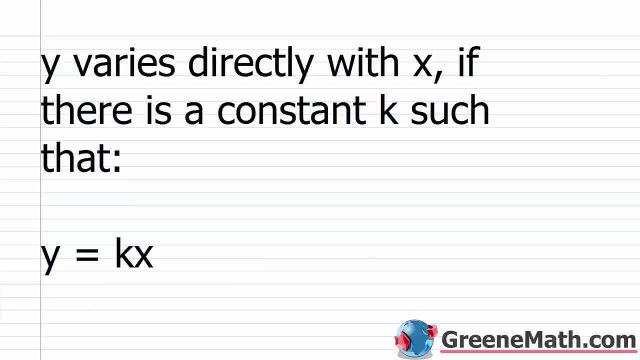 and then also inverse variation which we're going to cover 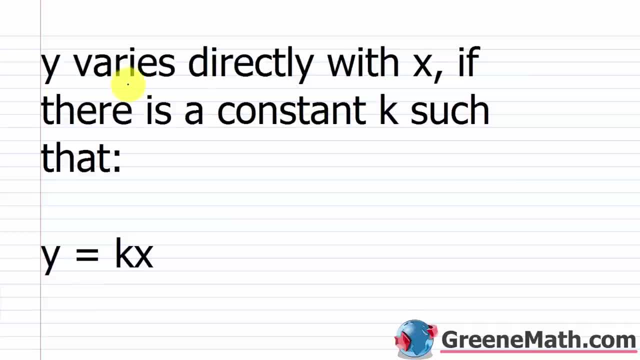 in the next lesson so I want to just start out by saying y varies directly with x if there is a constant k such that y is equal to k times x now this is generally the first thing 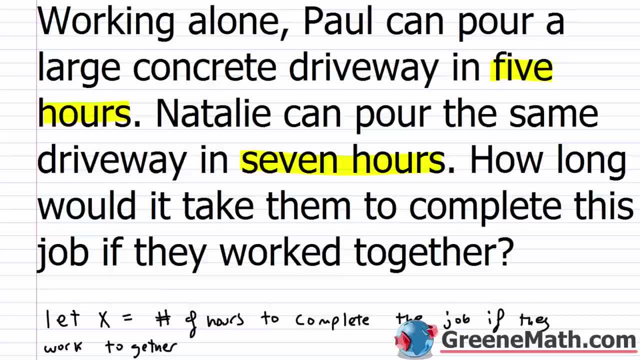 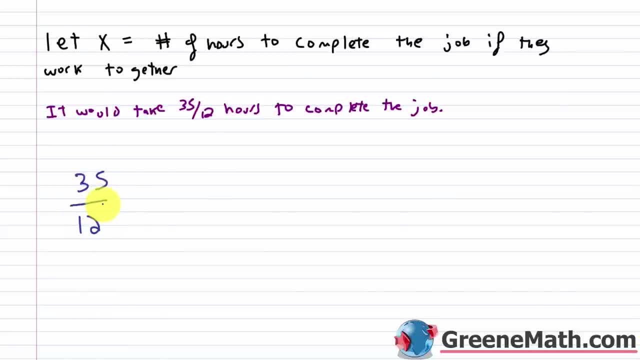 How long would it take for them to complete this job If they work together? So what I am going to do here Is I am going to take thirty five twelfths, Thirty five twelfths, Which is the number of hours they work for. 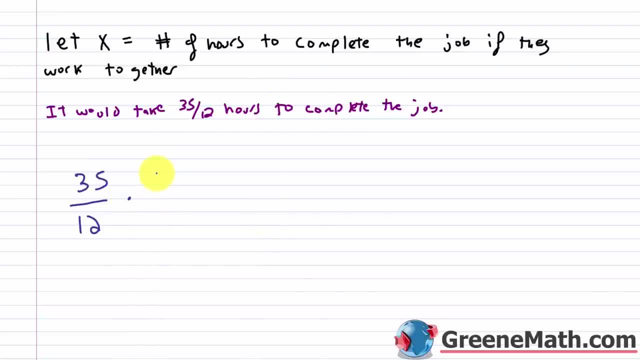 I am going to multiply this by The rate of speed that Paul works at, Which is one fifth, And then, plus I am going to do thirty five twelfths Times the rate of speed That Natalie works at, Which is one seventh. 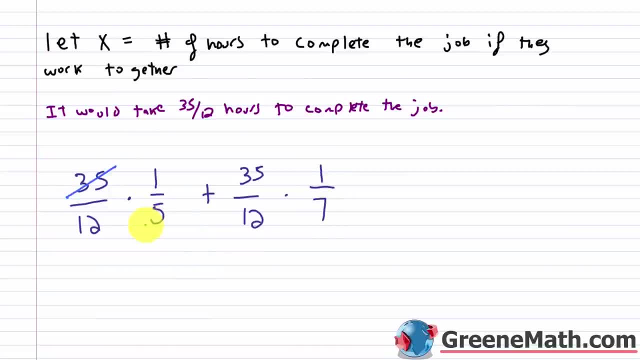 And let's see if this equals one. One completed job. This would give me seven, So I would have seven over twelve. So that means that in this amount of time, Thirty five twelfths Hours, Paul completes seven twelfths of that driveway. 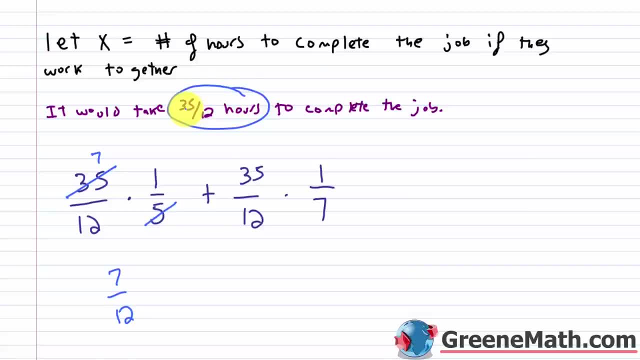 He completes seven twelfths of that job, You might want to say. And then Natalie's contribution Is less Because she works at a slower rate. This, divided by this, would give me five. She does five twelfths of the job. 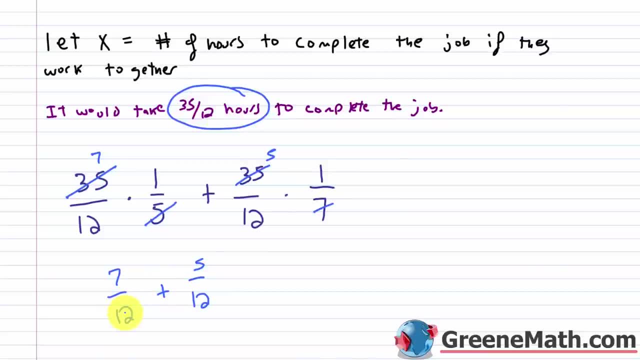 So, in this amount of time, Paul contributes seven twelfths, Natalie contributes five twelfths, Which equals what Seven plus five is twelve. Twelve over twelve is one, So they do complete one job. Hello and welcome to algebra. one lesson fifty. 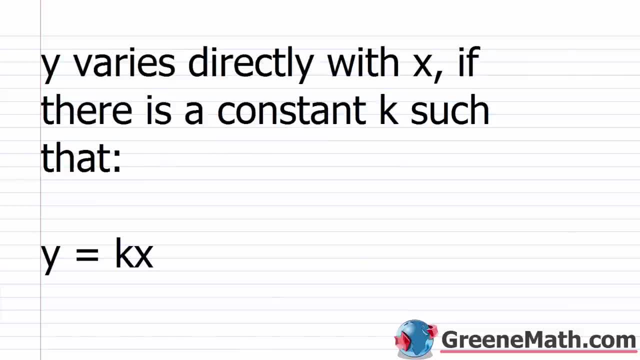 In this video we are going to learn about direct variation. So throughout your studies of algebra You are going to encounter many different types of variation. Obviously, as you move higher in algebra You get to algebra two And college algebra You know, so on and so forth. 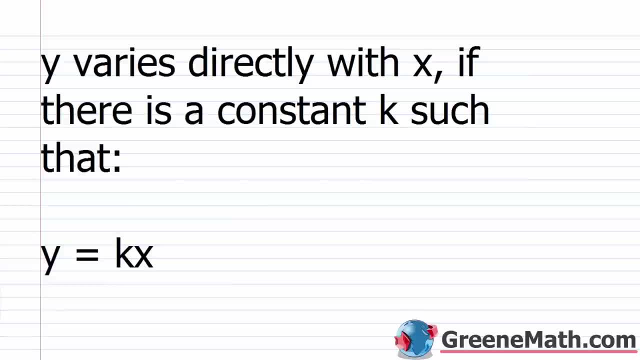 The types of variation that you are going to encounter Are going to become More challenging, But for an algebra one course, You are typically just going to deal with direct variation, Which we will see in this lesson, And then also inverse variation, 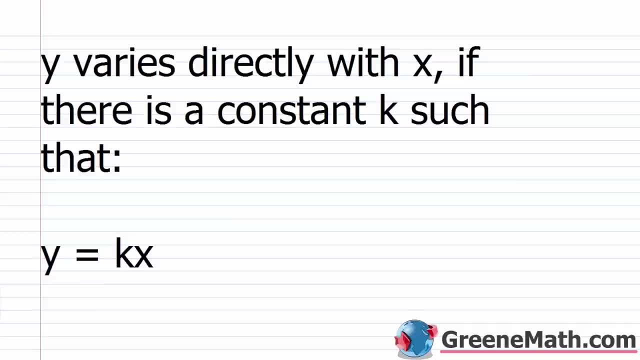 Which we are going to cover in the next lesson. So I want to just start out by saying: Y varies directly with X If there is a constant K, Such that Y is equal to K times X. Now, this is generally the first thing. 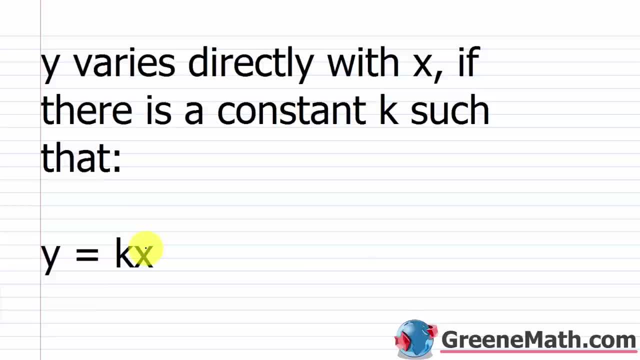 You are going to read in your textbook When you are in a direct variation section. So they have a special name. You are going to see this 4K. It is called the constant Of variation. Now, We have seen this type of equation before. 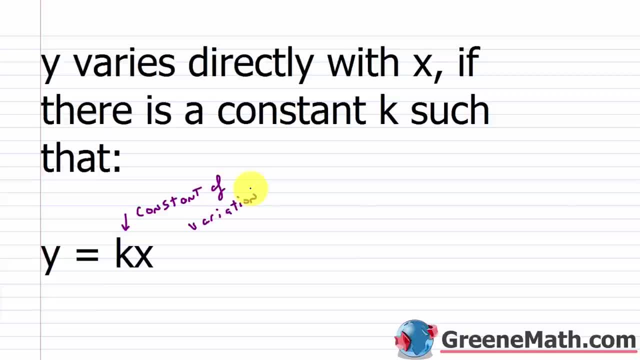 I want you to think back Many lessons ago When we learned about linear equations In two variables. Remember, we were graphing these things And we went through different forms of the line. And if I had a linear equation in two variables, 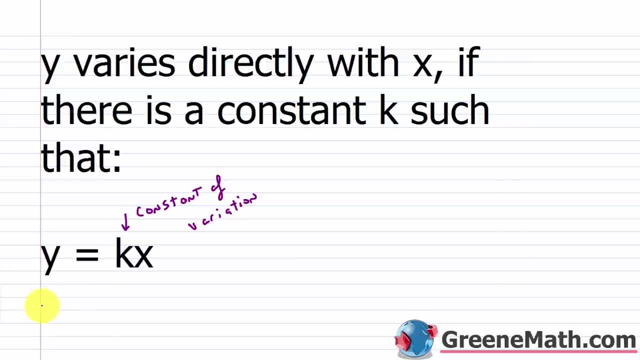 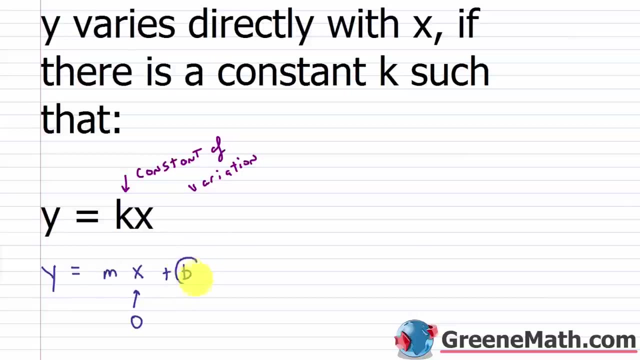 We would have a slope intercept form. We wrote this: as Y is equal to M, the slope Times X Plus B. Where B was the Y intercept? Remember I could plug in a zero for X And I would figure out What Y would be equal to. 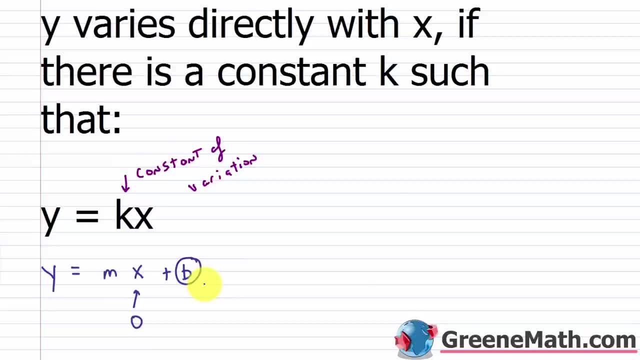 By just looking at what B was. So if I plugged in a zero for B, Let's say I had a zero for B And I had a Y intercept- That occurred at the point zero, comma zero. So plug in a zero for X. 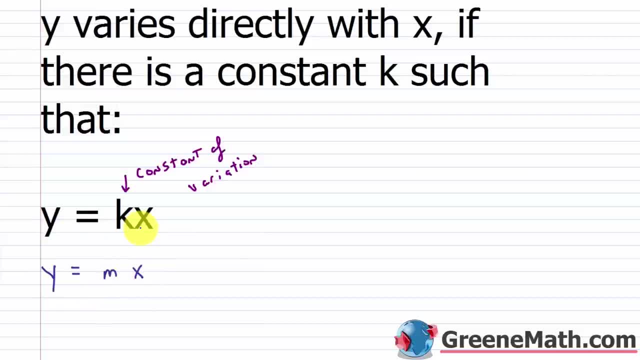 And a zero for Y. I have this exact equation here. It looks different Because this is an M And this is a K, But it is the same equation. I just swapped out letters And I renamed it. In this case, this is known as a slope. 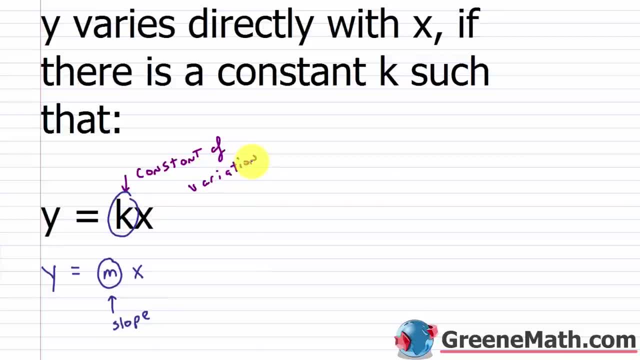 And when we get into the section on direct variation, We change it And we say it is the constant of variation. So, same equation, Same properties. One of the things you might remember: As X increases, So as X increases If K is positive. 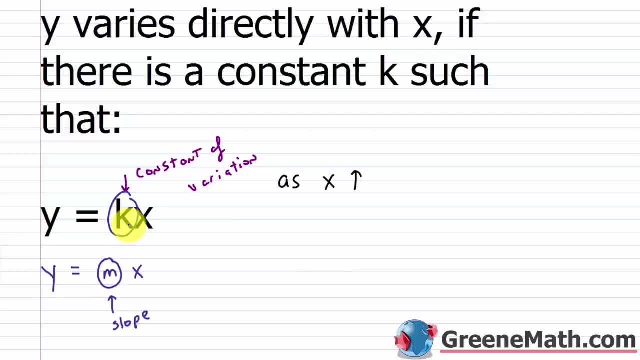 Then Y is going to increase. So if K- Let me write- If K is positive, As X increases, Y increases. But we can be more specific than that, Because as X, As X increases By one unit, We would see that 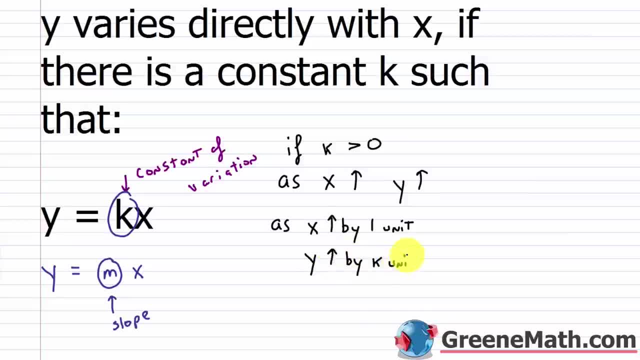 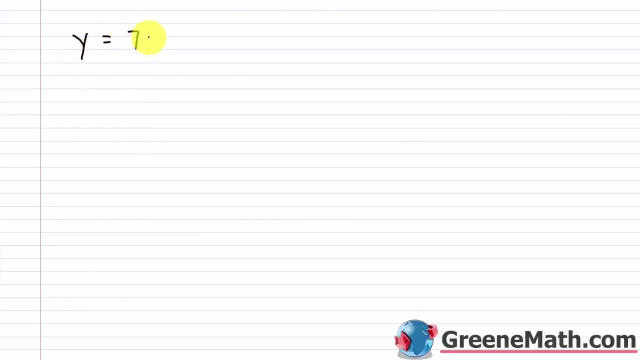 Y increases by K units By this constant of variation, That is multiplying X. Or again you can think about it as The slope. So to see an example of this, Let's just say we had something like Y equals 7X. 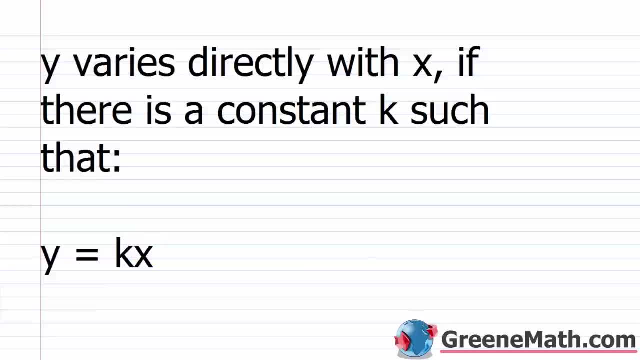 you're going to read in your textbook when you're in a direct variation section so they have a special name you're going to see this 4k it's called the constant constant of variation now we have seen 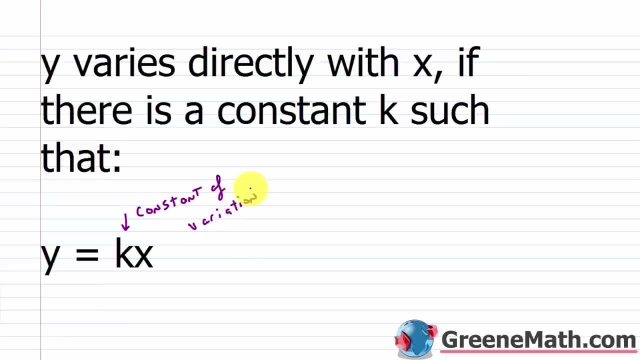 this type of equation before I want you to think back many lessons ago when we learned about linear equations in two variables remember we were graphing these things and we went through different forms of the line and if I had a linear equation in two variables in something known as slope intercept form we wrote this as y is equal to m the slope times x plus b where b was the y intercept remember I could plug in a 0 for x 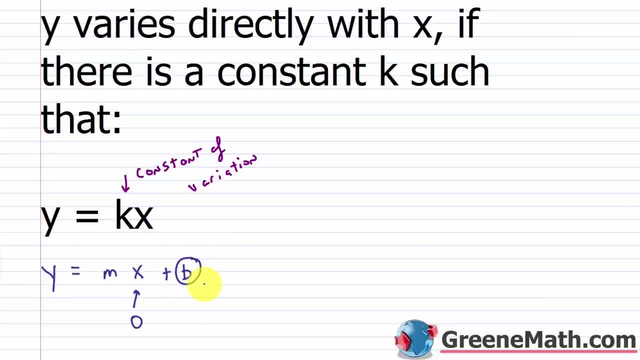 and I would figure out what y would be equal to by just looking at what b was so if I plugged in a 0 for b let's say I had a 0 for b and I had a y intercept that occurred at the point 0 comma 0 so plug in a 0 for x get a 0 for y I have this exact equation here it looks different because this is an m and this is a k but it's the same equation I just swapped out letters and I renamed it in this case this is known as a slope 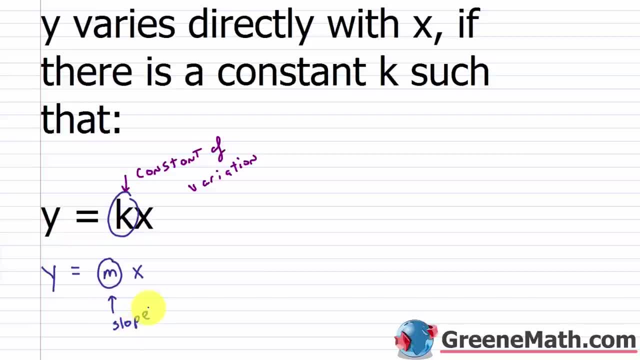 and when we get into the section on direct variation we change it and we say it's the constant of variation so same equation same properties one of the things that you might remember just to give you a little insight as x increases so as x increases 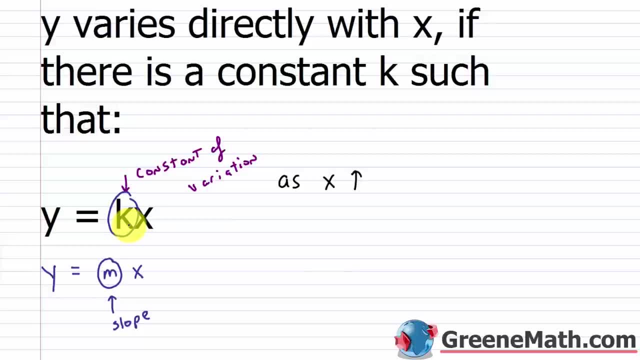 if k is positive then y is going to increase so if k let me write if k 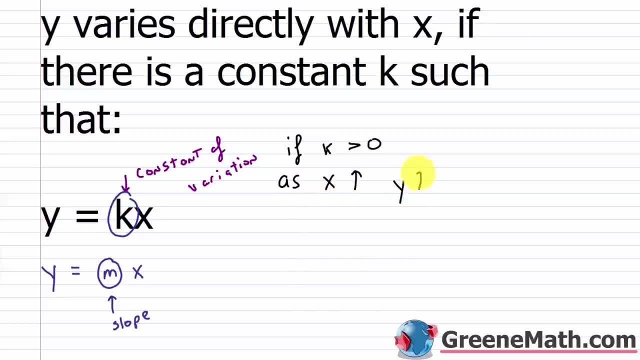 is positive as x increases y increases but we can be more specific than that because as x as x increases by one unit we would see that y increases by k units by this constant of variation that is multiplying x and we can think about it as the slope so to see an example of this let's just say we had something like y equals 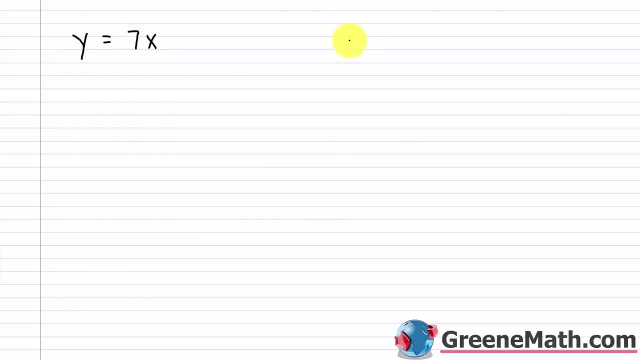 7x well if I started out by making like a little table let's say this is my x value this is my y value let's say I just start out by saying x is 1 so if x is 1 I plug in a 1 there 1 times 7 is 7 so y is 7 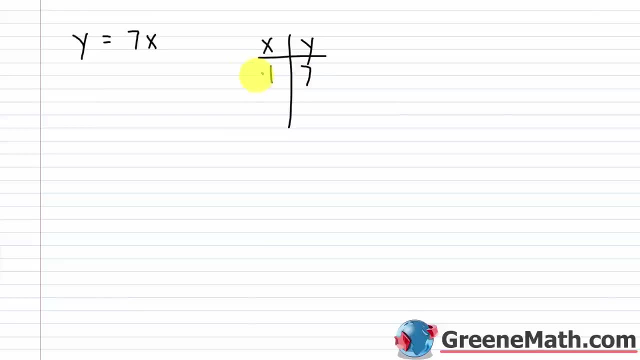 now as x increases by one unit so let me just say x is going to increase by one unit so this goes to 2 now what's y going to go to 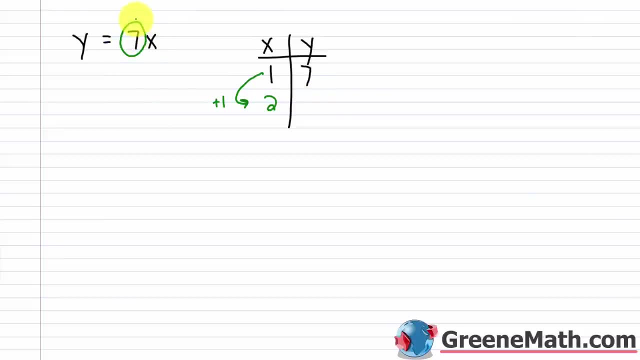 without plugging anything in I should know that y would increase by 7 units so 7 plus 7 is 14 so this should be 14 this increases by 7 units and does it plug in a 2 for x 2 times 7 is 14 so that is what you get again this is the case as you move up so if I go up by another 1 equals 3 now I would go up by another 7 so this would be y equals 21 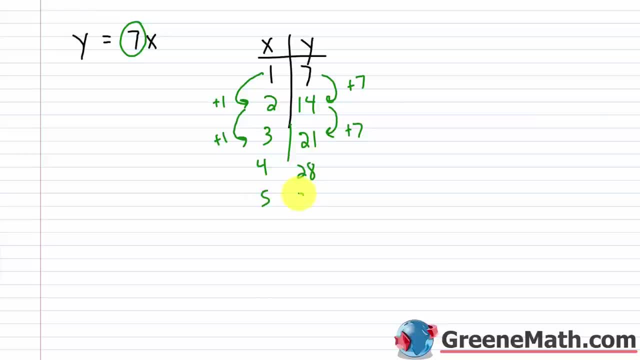 so if I did 4 this would be 28 if I did 5 this would be 35 so on and so forth 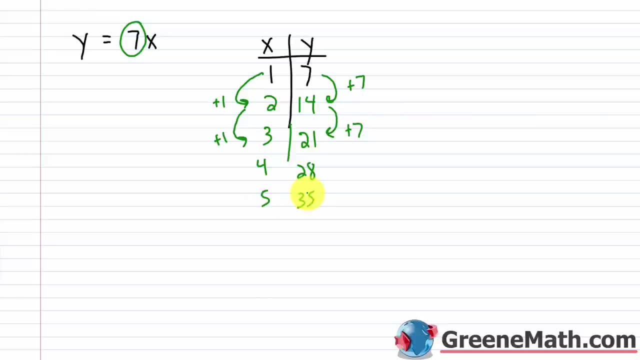 and this works in the opposite direction as well as I decrease x by 1 I'm decreasing y by 7 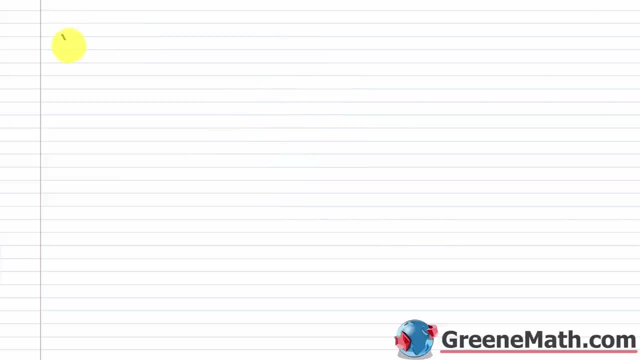 and to see that let's do another example let's say I had something like y equals 3x now so the constant of variation the k is 3 or I could say m is 3 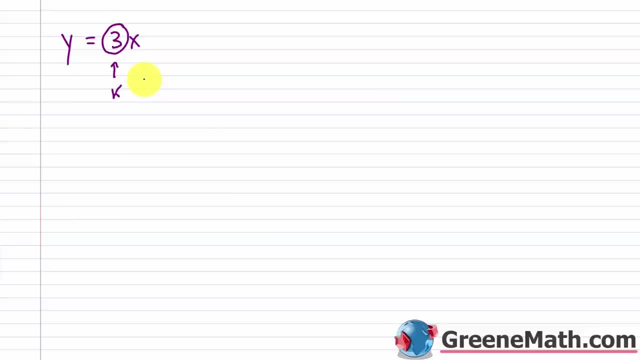 I could think of it as slope if that makes you feel more comfortable for right now 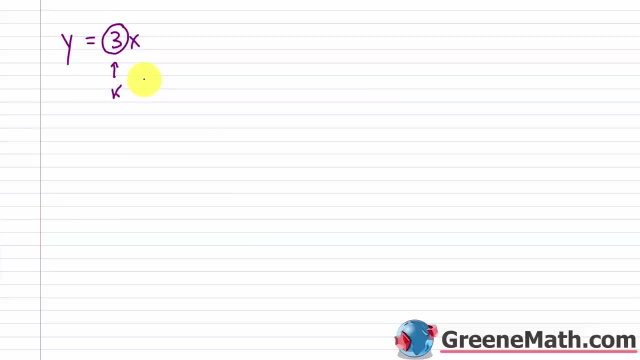 as I increase x by 1 unit y will increase by 3 units as I decrease x by 1 unit y will decrease by 3 units 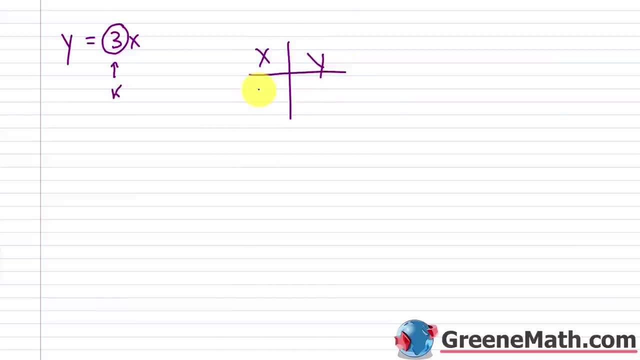 so in other words if I started out with let's say x equal to 10 so plug in a 10 for x 10 times 3 is 30 y would be 30 so I decreased x by 1 unit so let's say I went down to 9 I'm going to put minus 1 there 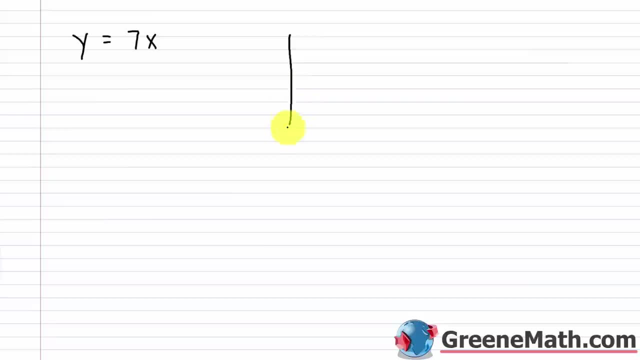 Well, if I started out By making like a little table, Let's say: this is my X value, This is my Y value. Let's say I just start out by saying X is 1.. So if X is 1. I plug in a 1 there. 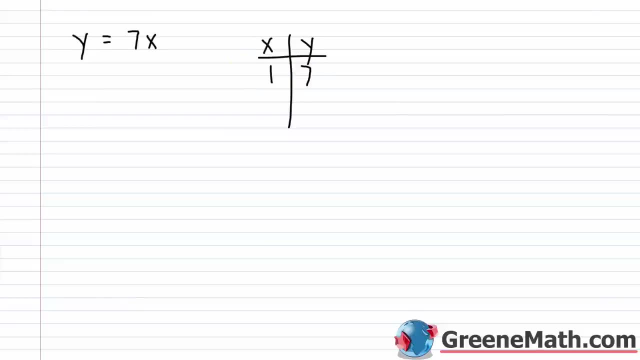 1 times 7 is 7.. So Y is 7.. Now, as X increases by one unit. So let me just say X is going to increase by one unit, So this goes to 2. now What is Y going to go to? 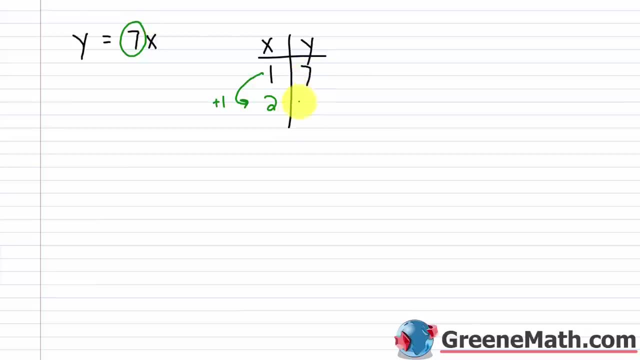 Without plugging anything in, I should know that Y would increase by 7 units. So 7 plus 7 is 14.. So this should be 14.. So if I plug in a 2 for X, 2 times 7 is 14.. 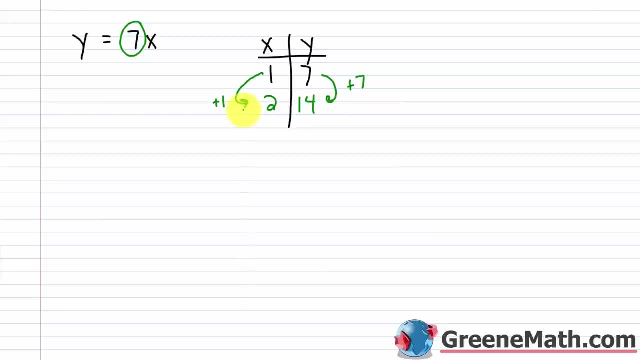 So that is what you get Again. this is the case as you move up. So if I go up by another 1. And this is X equals 3. now I would go up by another 7. So this would be Y equals 21.. 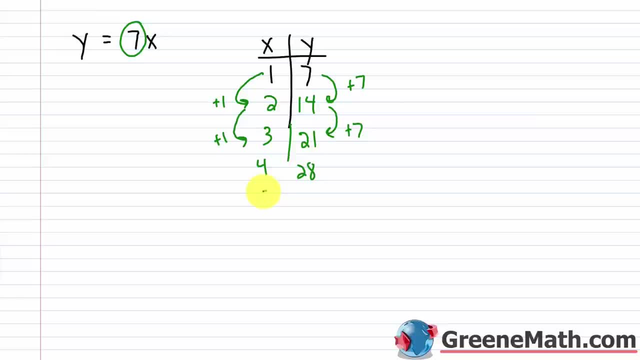 So if I did 4. This would be 28.. If I did 5. This would be 35. So on and so forth, And this works in the opposite direction as well. As I decrease X by 1. I increase Y by 7.. 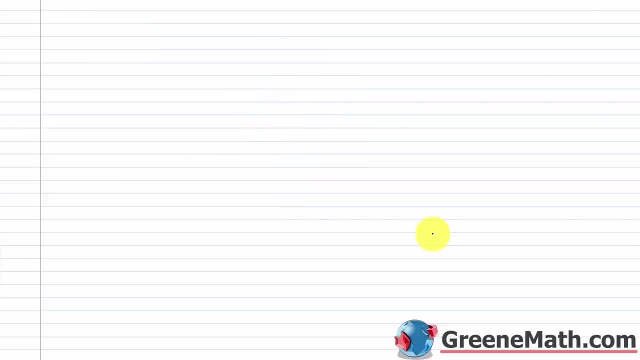 And to see that, Let's do another example. Let's say I had something like Y equals 3X now, So the constant of variation, The K, is 3.. Or I could say M is 3.. I could think of it as slope. 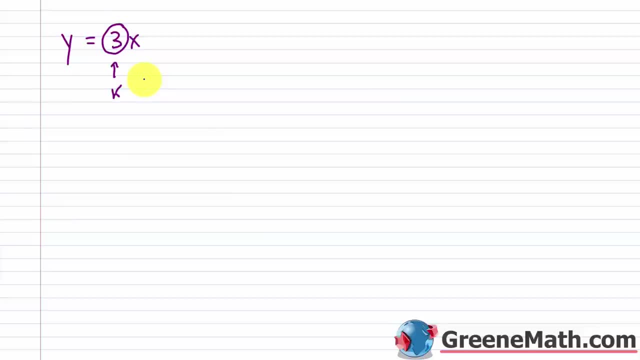 But that makes you feel more comfortable. for right now, As I increase X by 1 unit, Y will increase by 3 units. As I decrease X by 1 unit, Y will decrease by 3 units. So in other words, If I started out with, 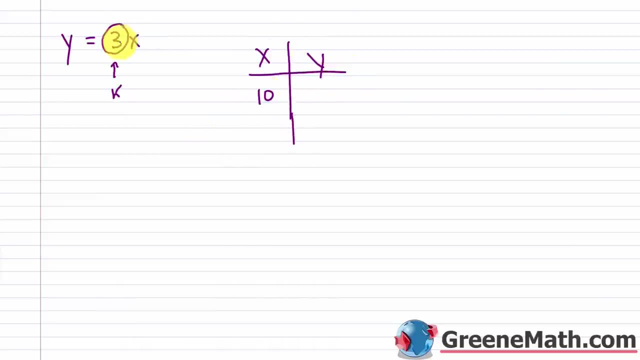 Let's say X equal to 10.. So plug in a 10 for X. 10 times 3 is 30. Y would be 30. If I decrease X by 1 unit. So let's say I went down to 9.. 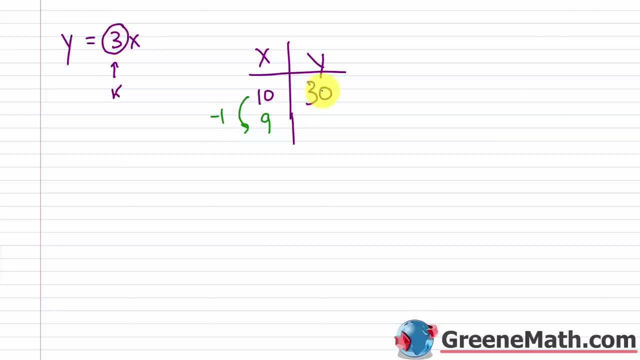 I'm going to put minus 1 there. Y is going to decrease by 3 units. So 30 minus 3 is 27.. And of course, if I plugged in a 9 there, 9 times 3 is 27.. 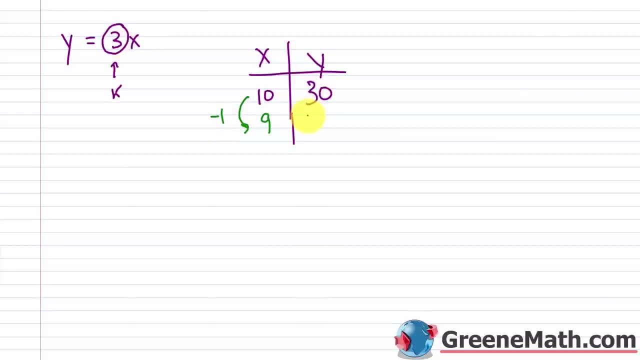 y is going to decrease by 3 units so 30 minus 3 is 27 and of course if I plug in a 9 there 9 times 3 is 27 so this decreases by 3 and you can keep going if I put an 8 here this would be 24 7 here this would be 21 6 here this would be 18 so every time I decrease x by 1 I am decreasing y by 3 that constant of variation or again that slope so it's simple enough to understand 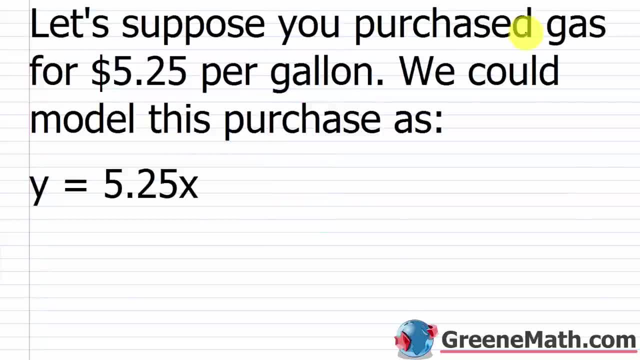 I want you to think about a real world scenario now let's suppose you purchased gas for $5.25 per gallon we could model this purchase as y which is the total the total cost or kind of your ending transaction is equal to 5.25 this is going to be your k your constant of variation or your slope however you want to think about that 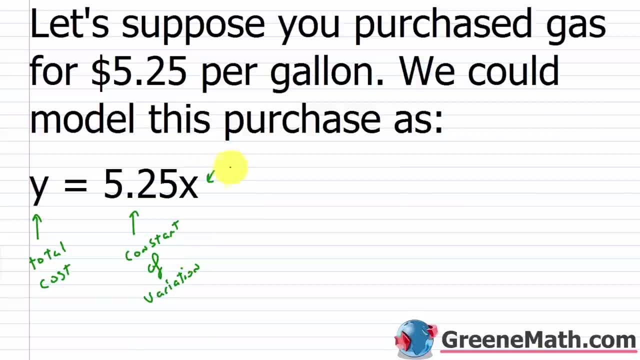 and then x is going to be the number of gallons purchased 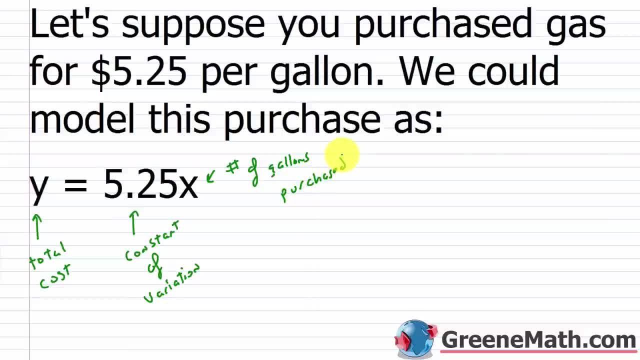 so we've all done stuff like this let's say you go up to the gas pump and you have let's say $20 in your wallet 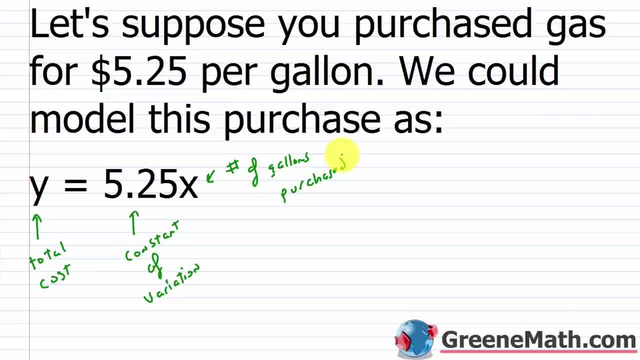 and it's $2 a gallon make it really really simple you know what to do you know that you can buy 10 gallons of gas you can't go over that because you only have $20 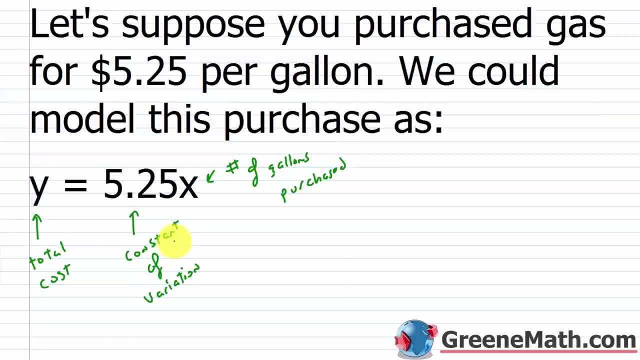 so it's the same thing here if we've modeled this purchase it's $5.25 per gallon of gasoline purchased well of course if I plug in a 1 there 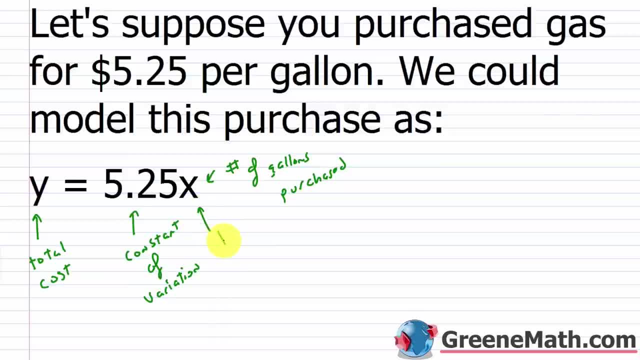 I'm going to pay $5.25 for that transaction if I plug in a 2 I just increase what I just had by 5.25 so now I'm paying $10.50 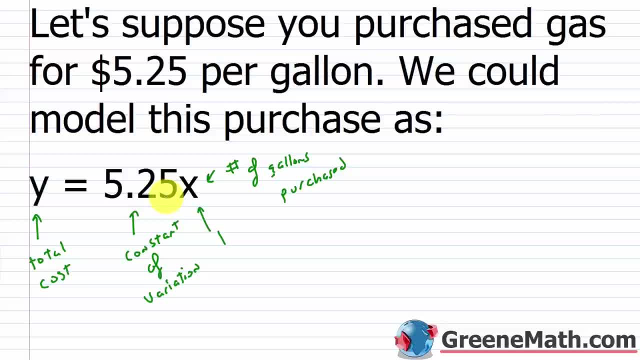 if I increase it to 3 or 5.25 so now I'm paying $15.75 or $15.75 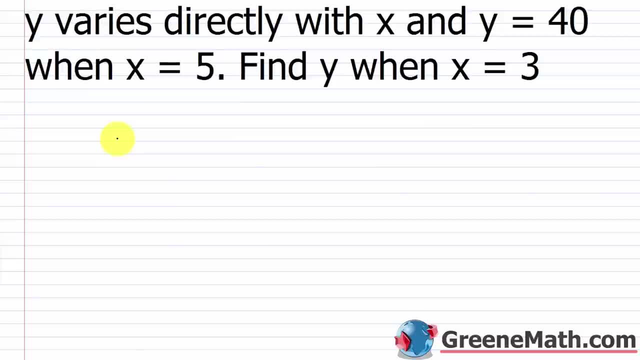 right so on and so forth alright so now that we have a little bit of understanding under our belts let's look at a typical problem that you're going to see 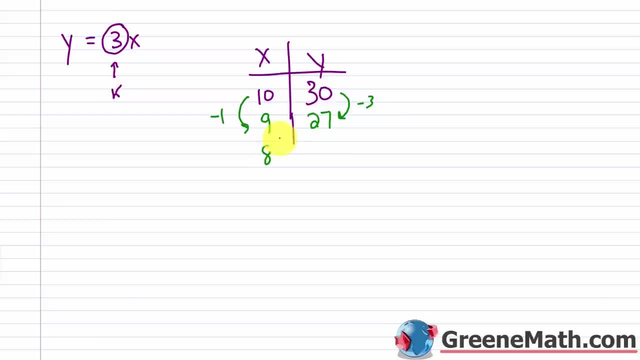 So this decreases by 3. And you can keep going. This would be 24.. 7 here, This would be 21.. 6 here, This would be 18.. So every time I decrease X by 1. I am decreasing Y. 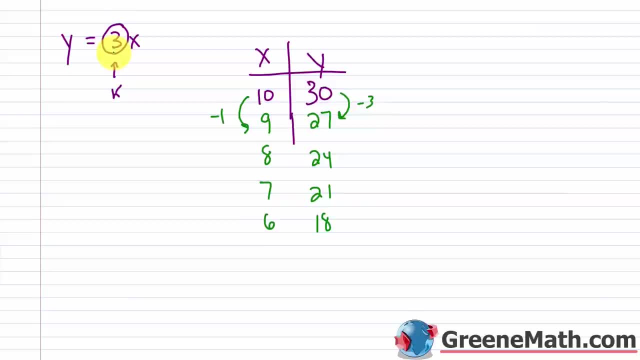 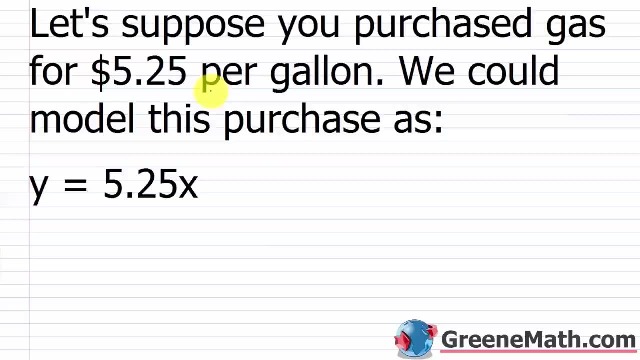 By 3. That constant of variation, Or again that slope. So that's simple enough to understand. I want you to think about a real world scenario now. Let's suppose you purchased gas For $5.25 per gallon. We could model this purchase. 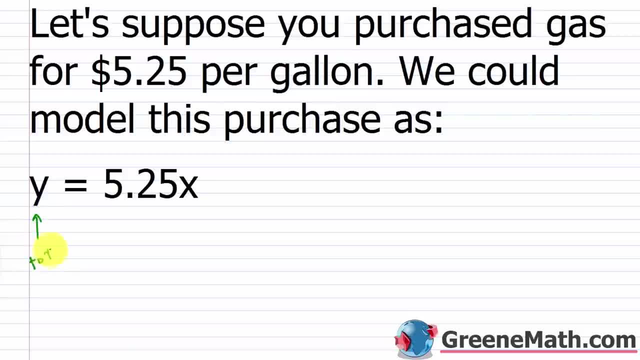 As Y, Which is the total. The total cost Or kind of your ending transaction Is equal to 5.25.. This is going to be your K, Your constant Of variation, Or your slope, Or however you want to think about that. 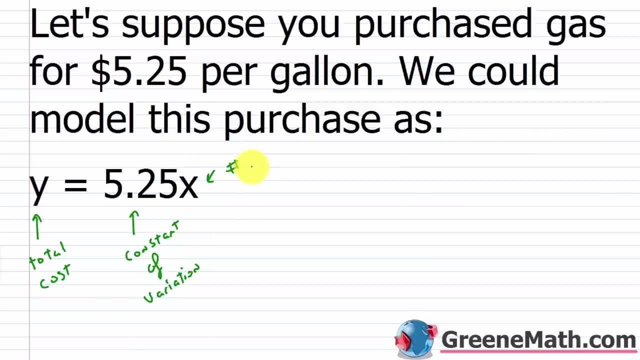 And then X Is going to be the number Of gallons Purchased. So we've all done stuff like this. Let's say you go up to the gas pump And you have, Let's say, $20 in your wallet And it's $2 a gallon. 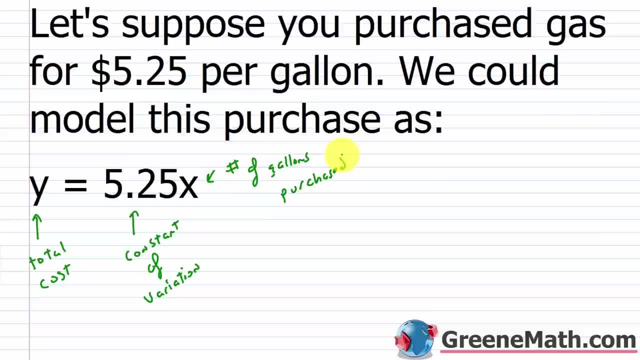 Make it really, really simple. You know that you can buy 10 gallons of gas. Can't go over that because you only have $20.. So it's the same thing here If we've modeled this purchase As $5.25.. 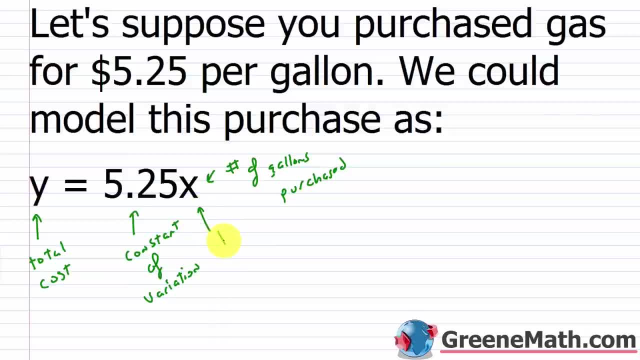 Per gallon of gasoline purchased. Well, of course, if I plug in a 1 there, I'm going to pay $5.25. For that transaction. If I plug in a 2. I just increase what I just had By $5.25. 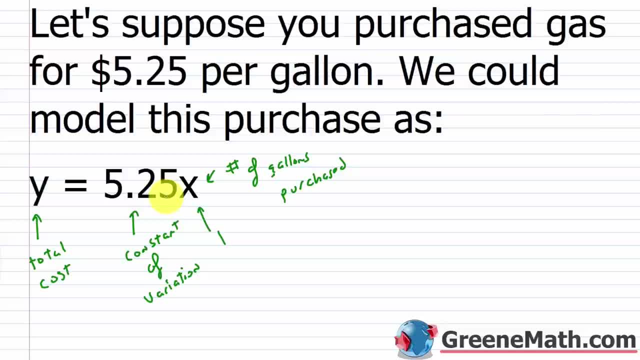 So now I'm paying $10.50.. If I increase it to 3. I go up by another $5.25.. So now I'm paying $15.75.. Or $15.75.. Right, so on and so forth. 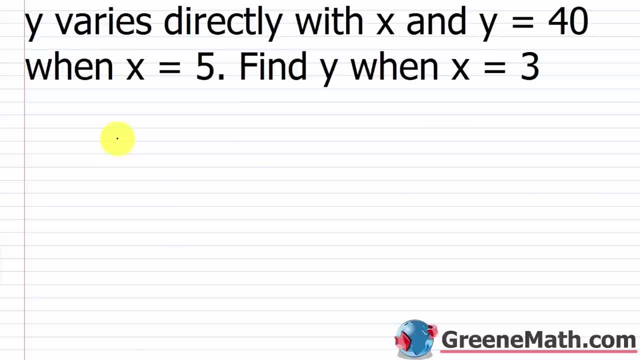 Alright, so now that we have a little bit Of understanding under our belts, Let's look at a typical problem that you're going to see, Kind of when you get to the questions In the back of your book Or for your homework. 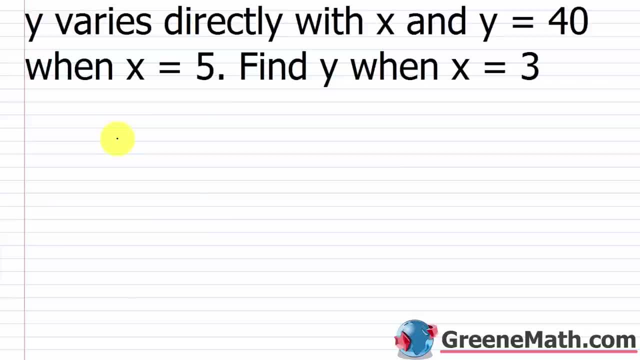 kind of when you get to the questions in the back of your book or for your homework or for a test and these type of scenarios are very very easy to deal with so we have that y varies directly with x 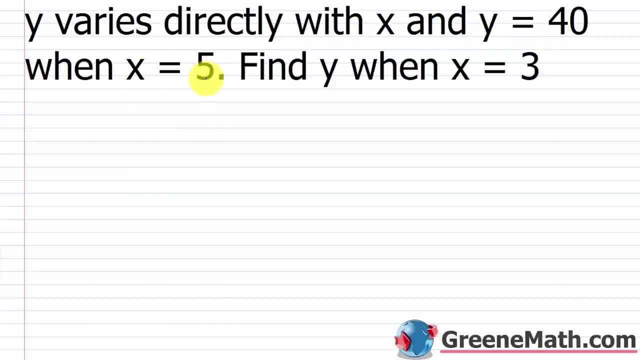 and y equals 40 when x equals 5 that's the first part 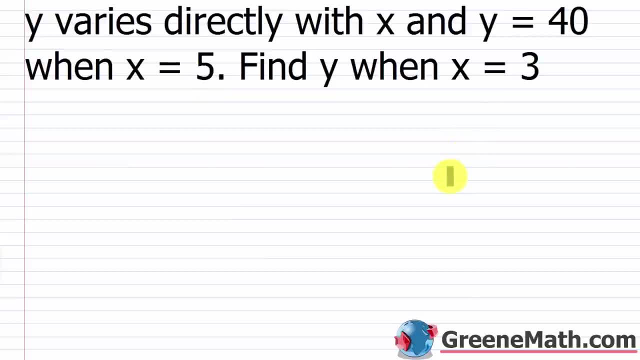 they kind of give you an opening case to deal with and then they're going to give you a problem to solve 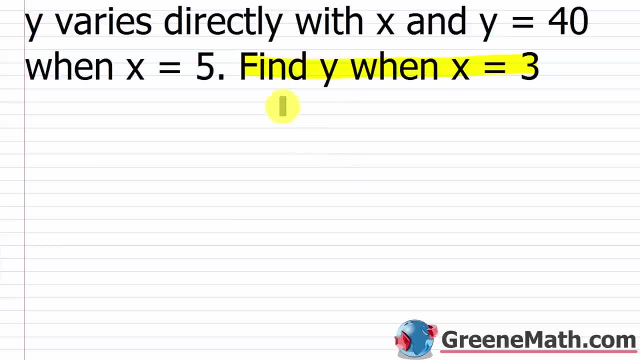 it says find y when x equals 3 so I'm not going to deal with this until last the first thing I'm going to always do is I'm going to find k the constant of variation in order to do that I need to do a little basic algebra so we say that again y varies directly with x and y equals 40 so I'm going to write this equation y equals kx that's my direct variation equation and then y they're saying is 40 so I'm going to plug in a 40 there 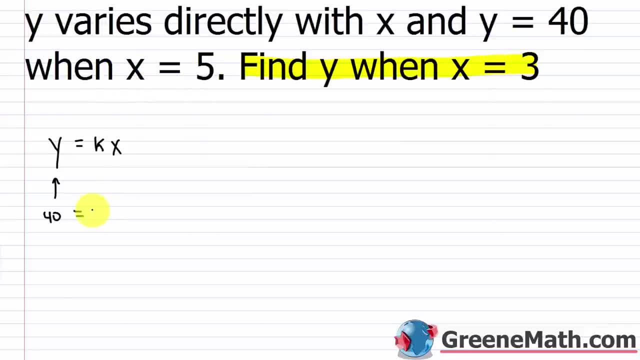 and that says when x equals 5 so I don't know what k is but I know x is 5 and to switch that around so it looks more traditional let's put 5k now how would I go about finding the value for k here well this is a linear equation in one variable and so all I need to do is divide both sides of the equation by 5 this is the coefficient for k and so this is going to cancel with this 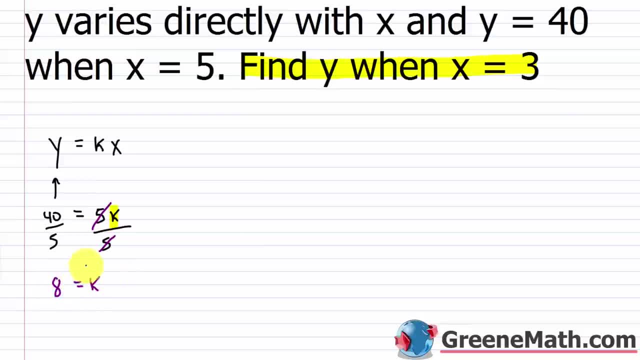 40 divided by 5 is 8 so I get 8 is equal to k so once I have found my constant of variation all I need to do is deal with this scenario that they're asking me to provide an answer for so it says find y when x equals 3 well I know that k is 8 and I know x is 3 so that's pretty simple in this equation I'm just plugging things in that's all I'm doing so I plugged in an 8 for k 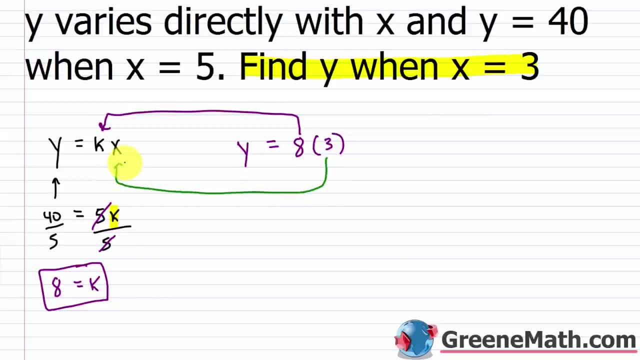 and I plugged in a 3 for x once I multiply these two together I'm going to find that y is equal to 24 so find y when x equals 3 again y is going to be equal to 24 and these problems are just that simple 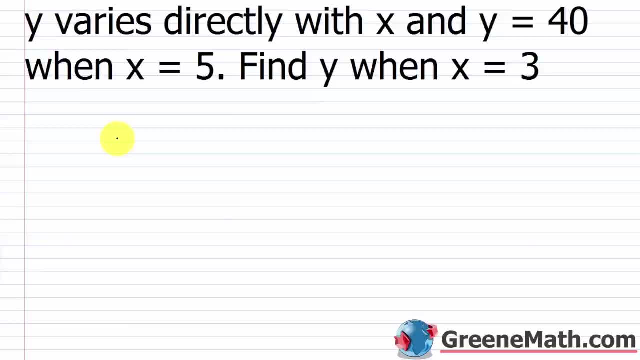 And these type of scenarios Are very, very easy to deal with. So we have that y varies directly with x And y equals 40. When x equals 5.. So that's the first part. They kind of give you an opening case to deal with. 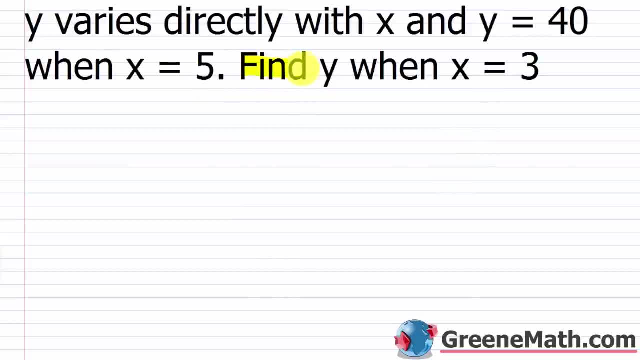 And then they're going to give you A problem to solve. It says find y when x equals 3.. So I'm not going to deal with this until last. The first thing I'm going to always do Is I'm going to find k. 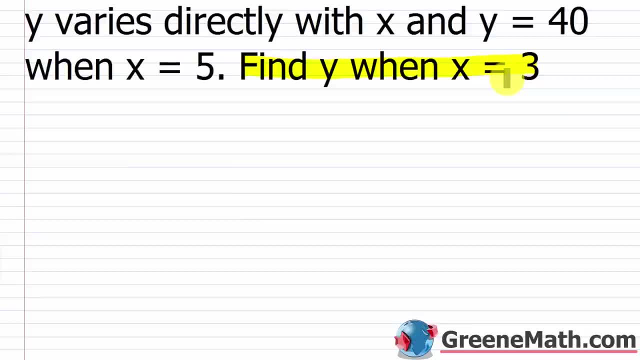 The constant of variation. In order to do that, I'm going to use a little basic algebra. So we say that again, Y varies directly with x And y equals 40. So I'm going to write this equation: Y equals kx. 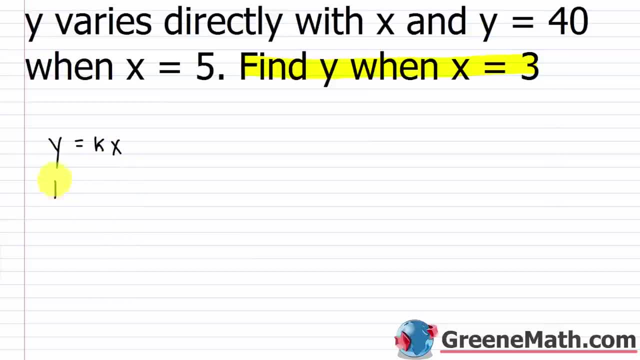 That's my direct variation equation. And then y they're saying is 40. So I'm going to plug in a 40 there And that says when x equals 5.. So I don't know what k is, But I know x is 5.. 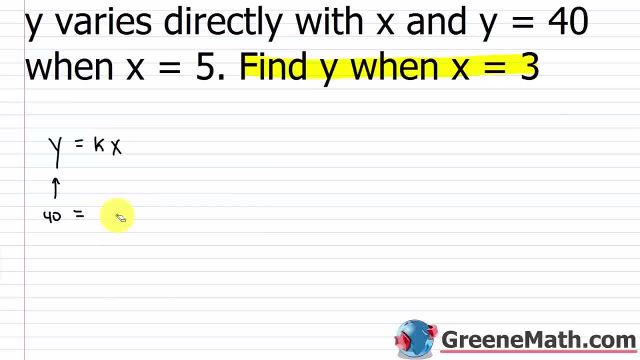 And to switch that around So it looks more traditional, Let's put 5k And then I go about finding the value For k here. Well, this is a linear equation In one variable, And so all I need to do is divide both sides. 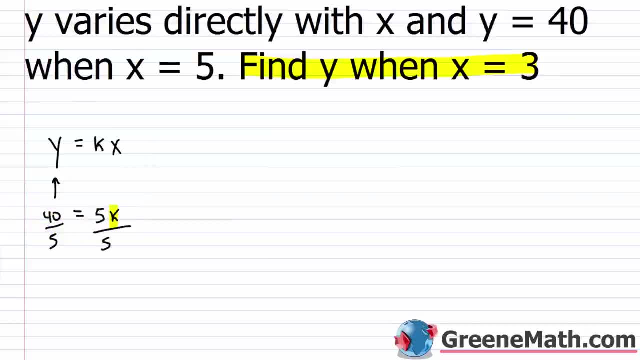 Of the equation by 5.. The coefficient for k- And so this is going to cancel with this- 40 divided by 5 is 8.. So I get: 8 is equal to k. So once I have found My constant of variation. 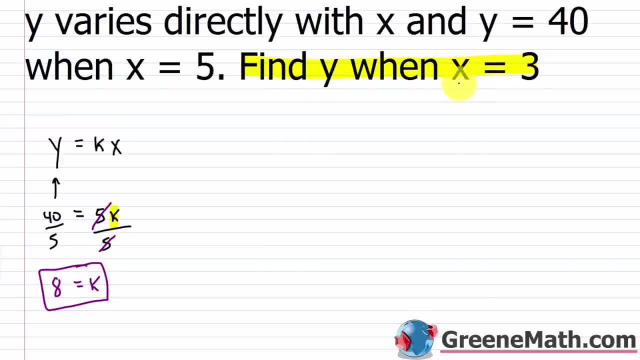 All I need to do is deal with this scenario That they're asking me To provide an answer for. It says: find y When x equals 3.. Well, I know that k is 8. And I know x is 3.. 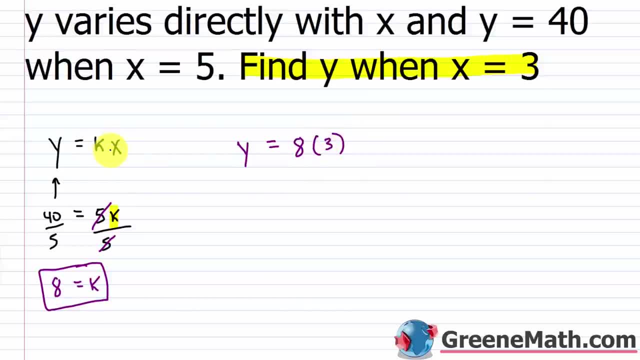 So that's pretty simple. I'm just following this equation. I'm just plugging things in, That's all I'm doing. So I plugged in an 8 for k And I plugged in a 3 for x. Once I multiply these two together. 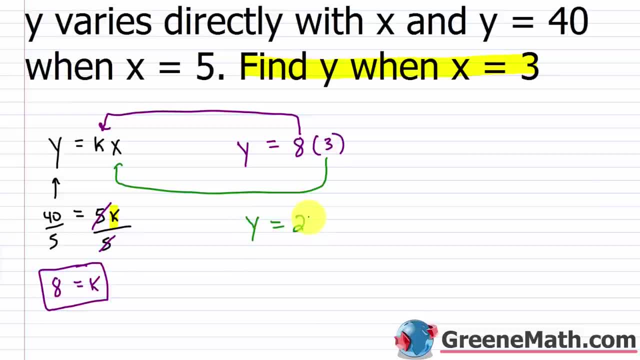 I'm going to find that y Is equal to 24.. So find y when x equals 3. Again, y is going to be equal to 24.. And these problems Are just that simple, Alright. so here's the next one. 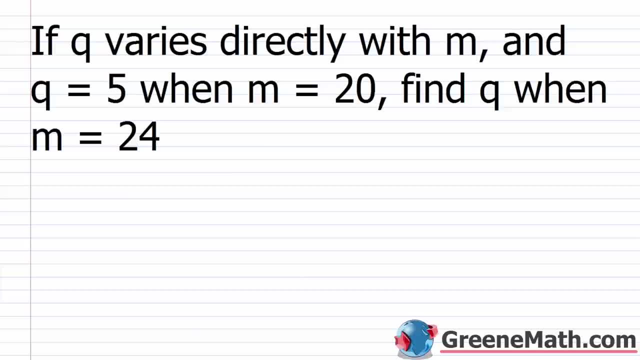 If q varies directly with m And q equals 5 when m equals 20.. Find q when m equals 24.. So you might see this And go: whoa, what's with all these letters? I'm very confused right now, But just follow the traditional. 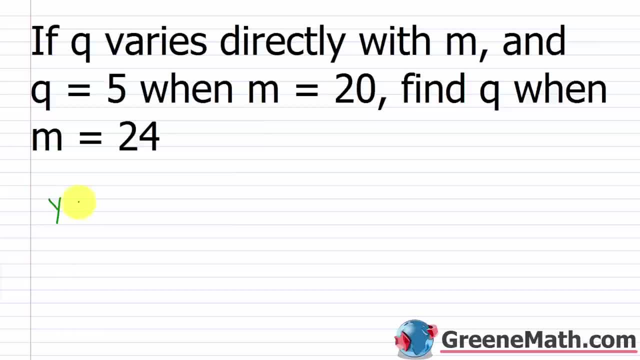 Format of x and y. So just start out with what you know: Y is equal to k times x. Okay, And q? that's varying directly with m. So this would be. In this scenario, Q would take the place of y. 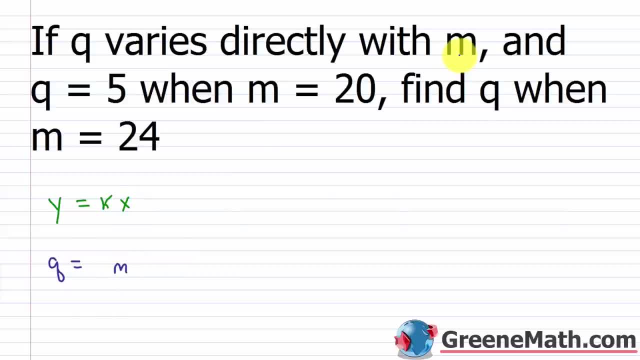 And m would take the place of x, And I know that could get extra confusing, Because we use m to denote slope And you have this k here Which is, you know, the same thing as slope. So just focus on what you're given. 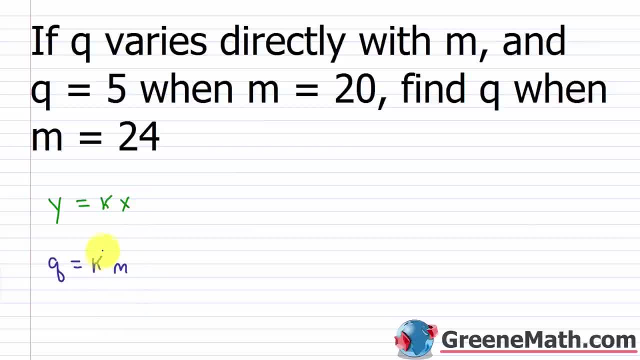 And take it piece by piece. I'm going to use m to represent x here And put my k there, And then I'm given information: Q equals 5. And m equals 20. So m is going to be a 20.. 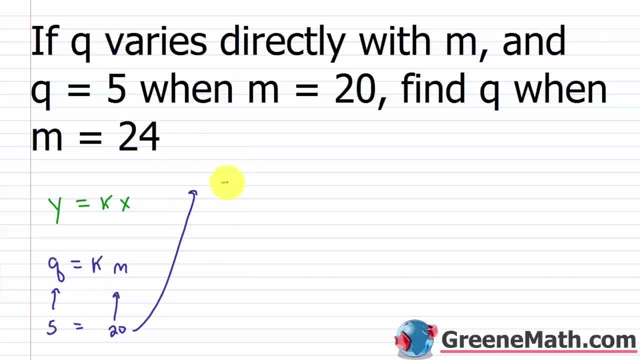 Very, very easy to solve. So let me drag this up here. And what would we have? 5 is equal to 20 times k. Divide both sides of the equation by 20.. So I can isolate k And we're going to do some canceling. 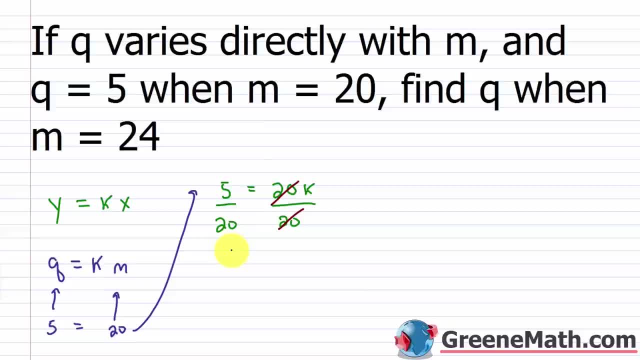 This would cancel with this And you get k equals 5 over 20.. 5 over 20 simplifies to 1 fourth, So 1 fourth is equal to k. So, now that I've found this information, My constant of variation. 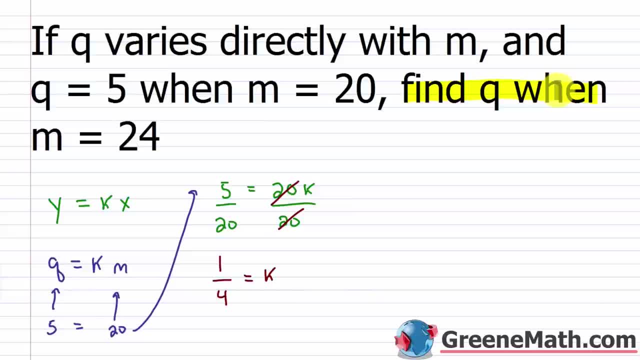 I have this scenario that they want me to deal with, Which is to find q When m equals 24.. So, using this equation that I've already figured out, I'm just going to plug in- I'm going to find q. So what is q? 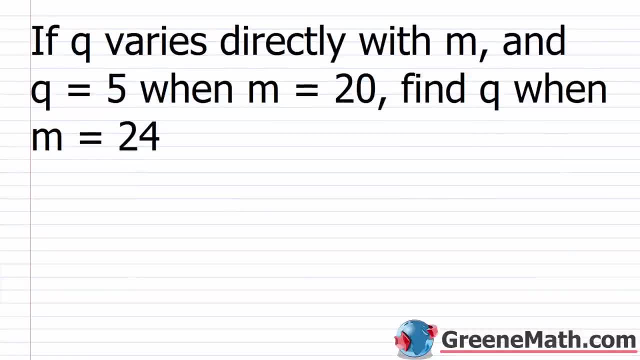 alright so here's the next one if q varies directly with m and q equals 5 when m equals 20 find q when m equals 24 so you might see this and go woah what's with all these letters 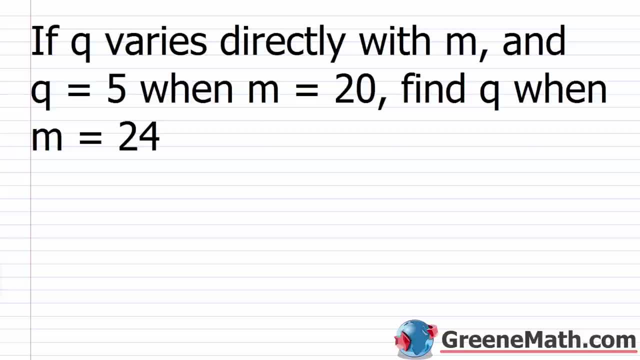 I'm very confused right now just follow the traditional format of x and y so just start out with what you know y is equal to k times x so now it's q that's varying directly with m so this would be in this scenario q would take the place of y and m would take the place of x and I know that could get extra confusing because we use m today to denote slope and you have this k here which is the same thing as slope 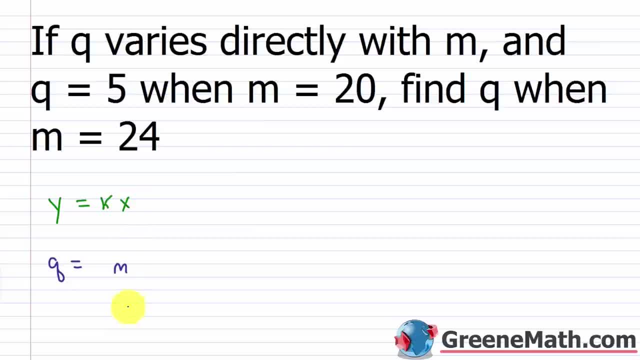 so just focus on what you're given and take it piece by piece I'm going to use m to represent x here and put my k there and then I'm given information q equals 5 so this is going to be a 5 when m equals 20 so m is going to be a 20 very very easy to solve so let me drag this up here divide both sides of the equation by 20 so I can isolate k and we're going to do some canceling this would cancel with this 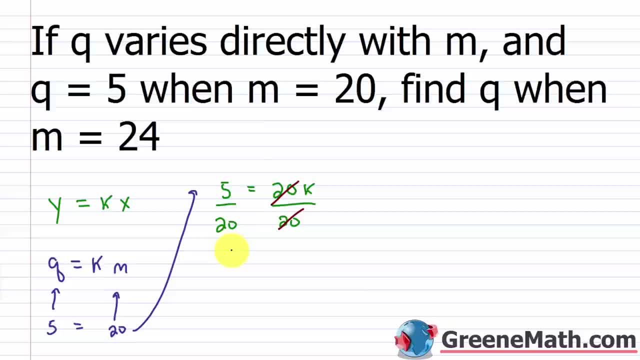 and you get k equals 5 over 20 5 over 20 simplifies to 1 fourth so 1 fourth is equal to k so now that I've found this information my constant of variation 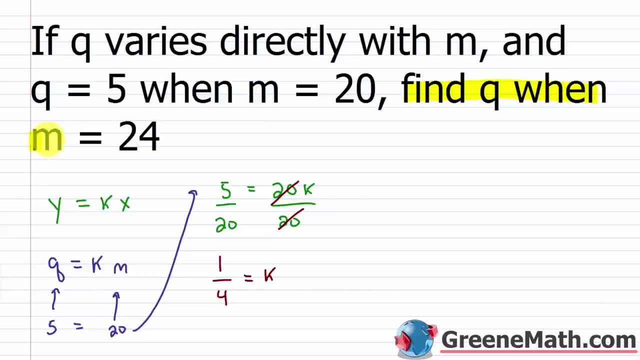 I have this scenario that they want me to deal with which is to find q when m equals 24 so using this equation that I've already figured out I'm just going to plug in I'm going to find q so what is q 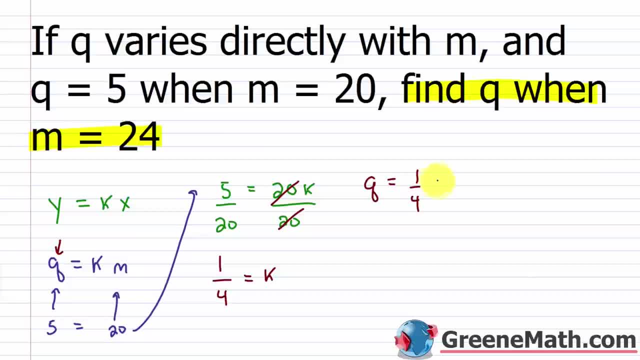 when m is 24 so I know k is 1 fourth 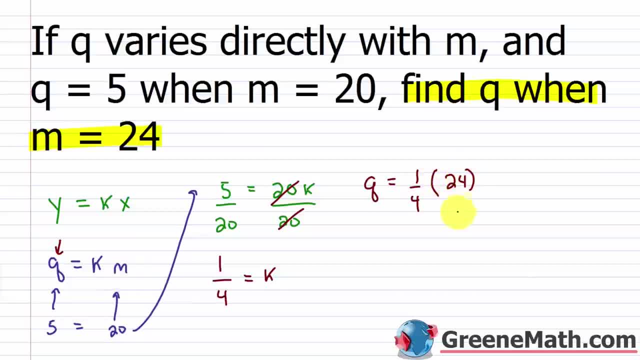 and I know that m is 24 multiply the two together 1 fourth times 24 is 6 because 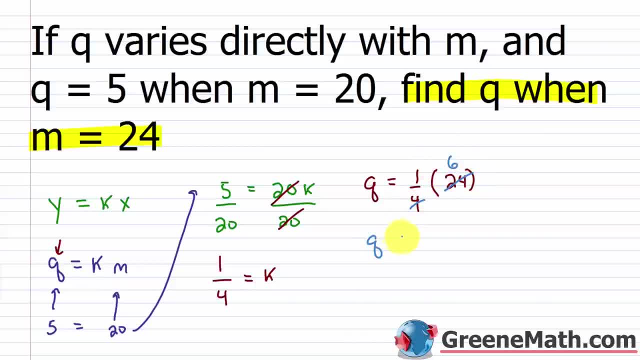 this would cancel with this and give me 6 6 times 1 is 6 so q equals 6 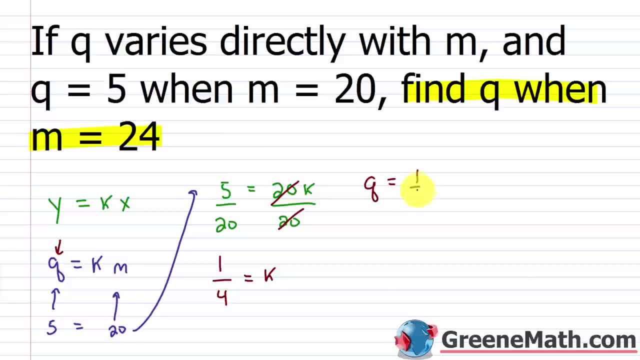 When m is 24.. So I know k is 1, fourth And I know that m is 24.. Multiply the two together: 1 fourth times 24 is 6.. Because this would cancel with this And give me 6.. 6 times 1 is 6.. 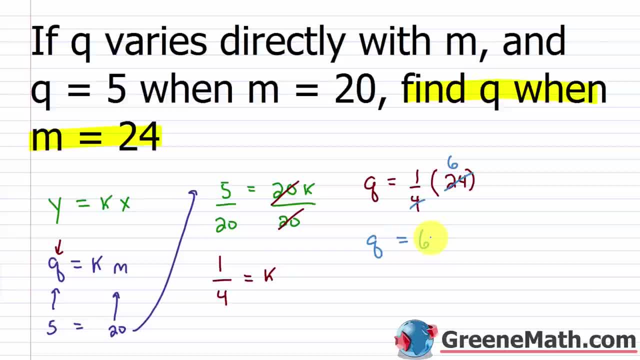 2 equals 6.. And again What I try to do in these scenarios Where they change the letters around- And typically you don't see this until you get to algebra 2. But I try to just replace it with what I know. 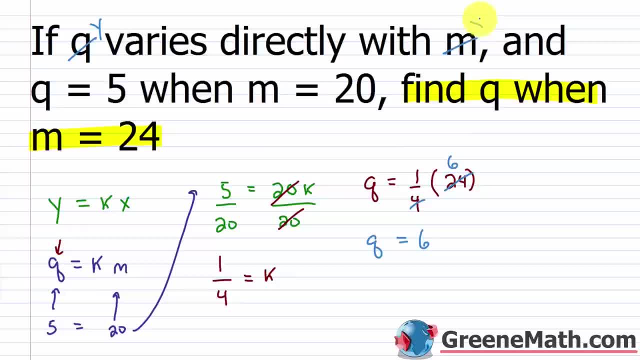 So I would say, okay, If y varies directly with x And y equals 5. When x equals 20. Find y When x equals 24.. So I would plug in All the information To my original formula And solve it. 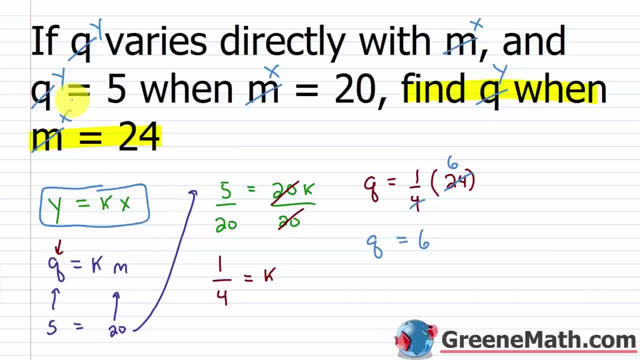 And then just go back And say: okay, Well, y was representing q, So y equals 6, is the answer I got, So q equals 6.. So on and so forth. That's how you deal with these letter changes When you first get them. 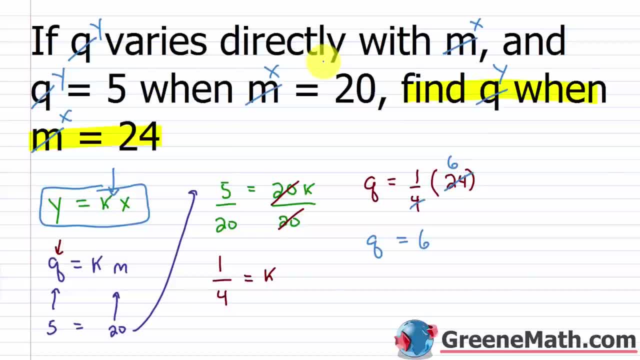 Because this is something you might see on the SAT Or the ACT And it's just them throwing a wrench at you Because they know that you've prepared for this, But they want to see if you can adapt And apply your knowledge. 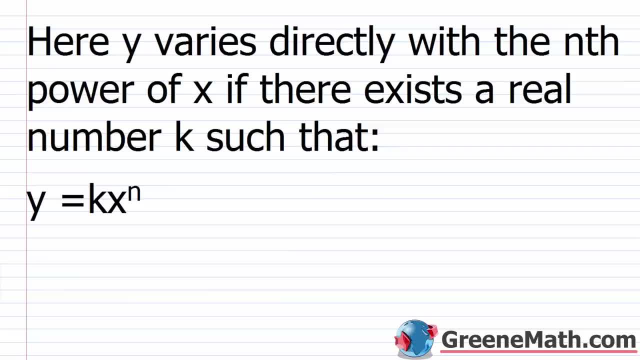 When you get a minor scenario change. So, now that we've dealt with two basic scenarios With direct variation, You're going to encounter something known as direct variation As a power. So it's not more difficult. You follow the same process to get your solution. 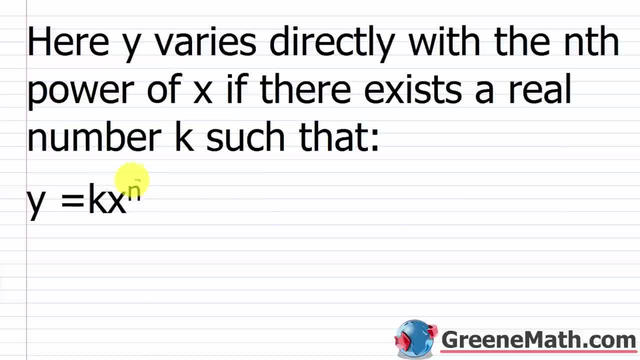 But you're just going to have a power On your variable x now. Okay, so Y is equal to k. Again, the constant of variation Times x raised to the nth power. So I have here: Y varies directly with the nth power of x. 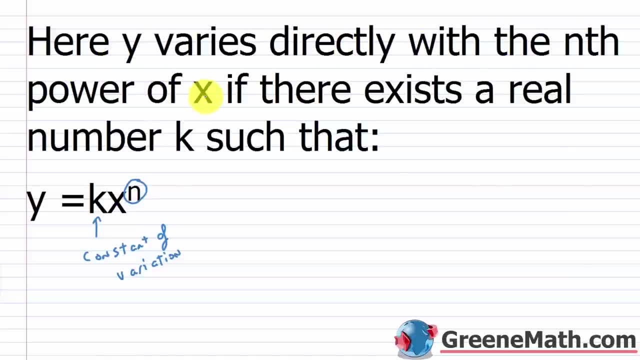 If there exists a real number, k, Such that again Y equals k, That constant of variation Times x raised to the nth power. So let's take a look at an example. here We have: If y varies directly with x squared, 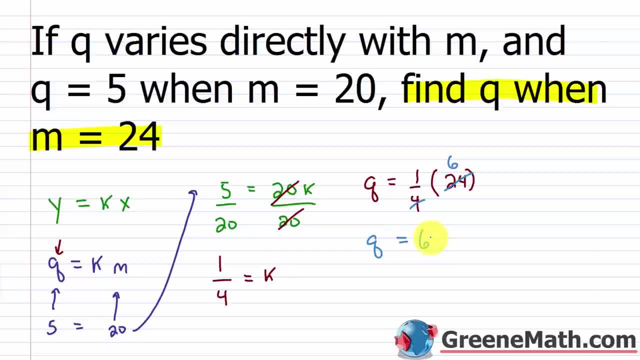 and again what I try to do in these scenarios where they change the letters around typically you don't see this until you get to algebra 2 but you can replace it with what I know so I would say 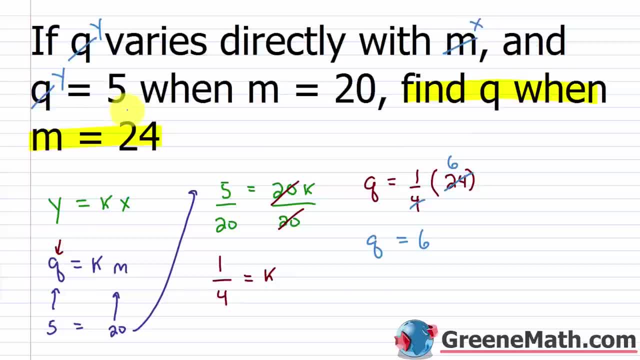 if y varies directly with x and y equals 5 when x equals 20 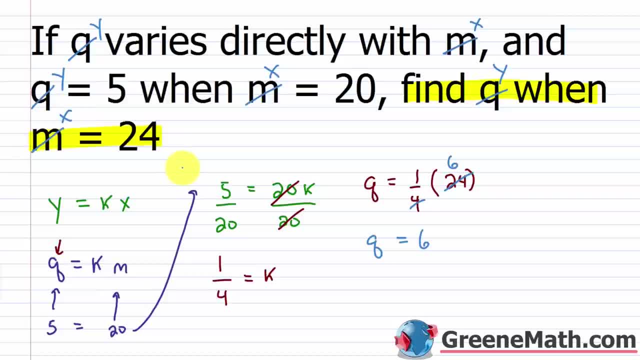 find y when x equals 24 find y when x equals 24 so I would plug in all the information 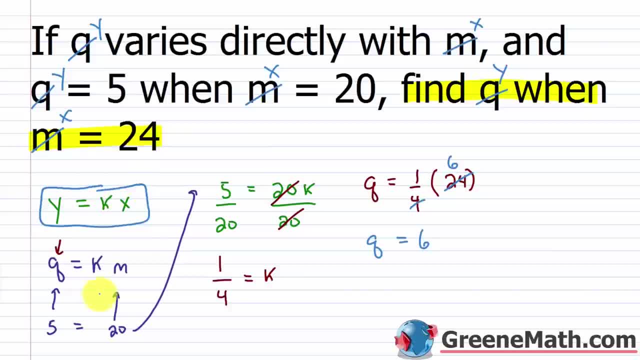 to my original formula solve it and then just go back and say y was representing q 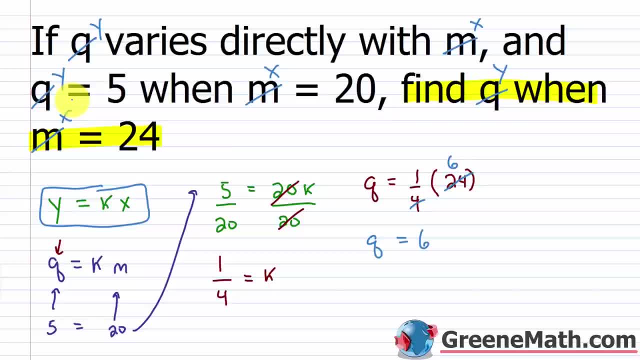 so y equals 6 is the answer I got so q equals 6 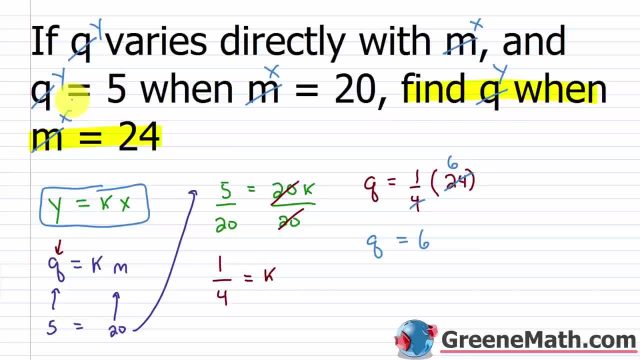 so on and so forth but this is something you might see on the SAT or the ACT and it's just them throwing a wrench at you 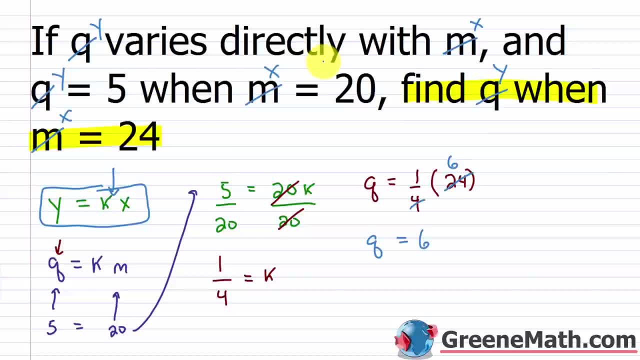 because they know that you've prepared for this but they want to see if you can adapt if you can go further than basically just regurgitating what you've learned in a textbook and kind of apply your knowledge when you get a minor scenario change 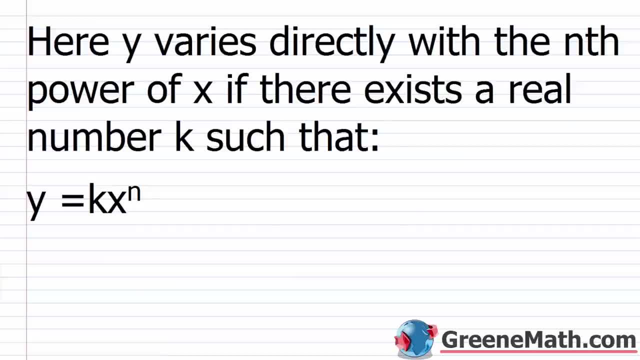 so now that we've dealt with two basic scenarios with direct variation 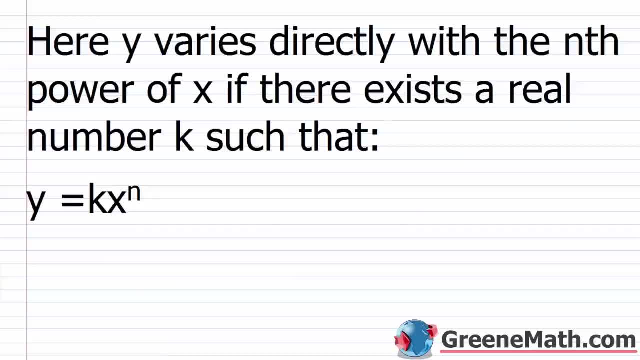 you are going to encounter something known as direct variation as a power more difficult. You follow the same process to get your solution. But you're just going to have 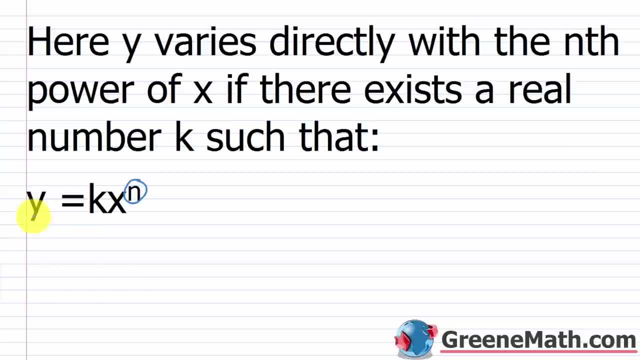 a power on your variable x now. Okay, so y is equal to k, again, the constant of variation, times x raised to the nth power. So I have here y varies directly with the nth power of x, 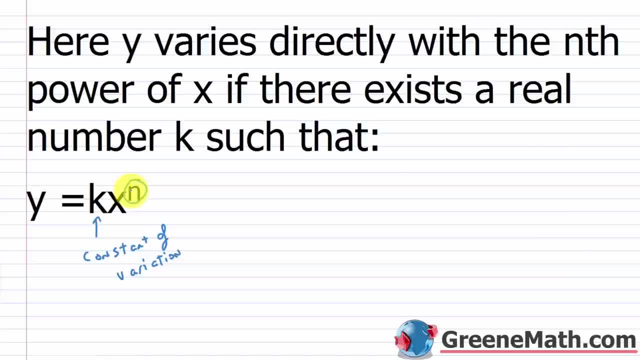 if there exists a real number k such that, again, y equals k, that constant of variation, 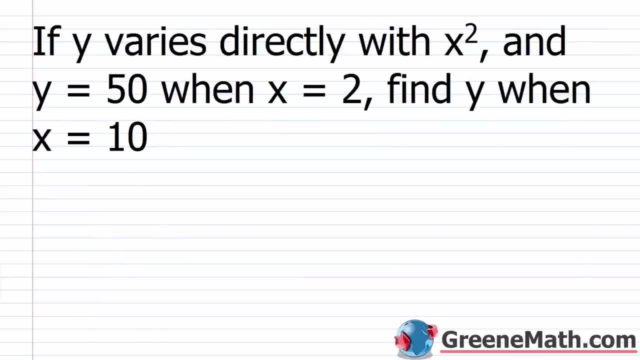 times x raised to the nth power. So let's take a look at an example here. We have if y varies 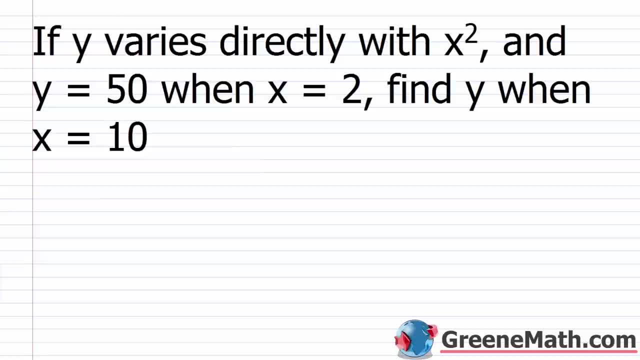 And y equals 50.. When x equals. 2. Find y when x equals. 3. Find y when x equals. 4. Find y when x equals. 5. Find y when x equals. 6. Find y when x equals, 7.. 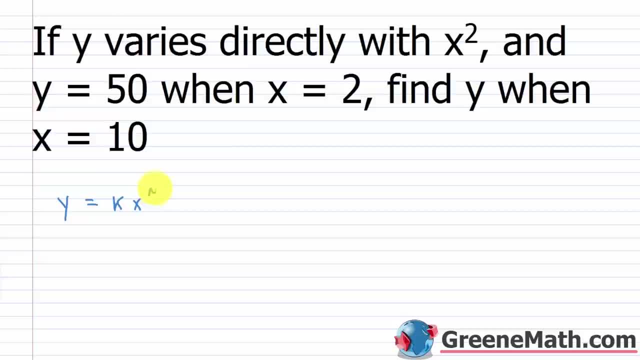 Find y when x equals. 8. Find y when x equals. 9. Find y when x equals 10.. So the equation with direct variation as a power, We just write that Y is equal to K times x to the nth power. 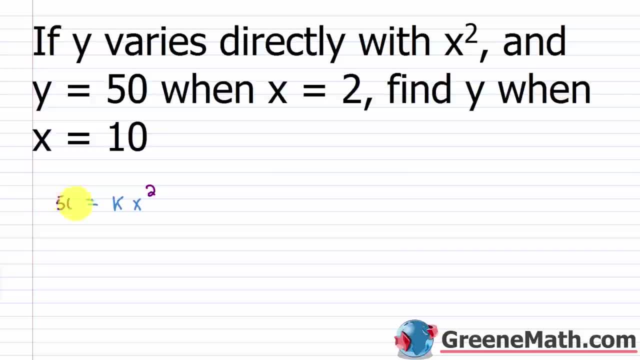 We're just going to plug in. It's just that simple. So if y varies directly with x, squared. So instead of an n I'm going to put a 2. there, Y equals 10.. So let's find k first. 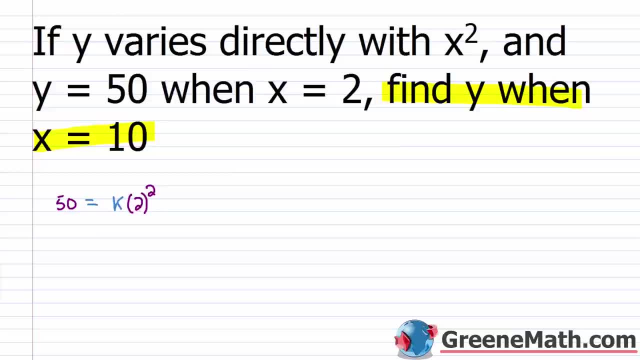 And then we'll deal with this scenario. Second: Okay, So 2 squared is obviously 4.. So you would get: 50 is equal to 4k. Divide both sides of the equation by 4.. And 50 is not divisible by 4.. 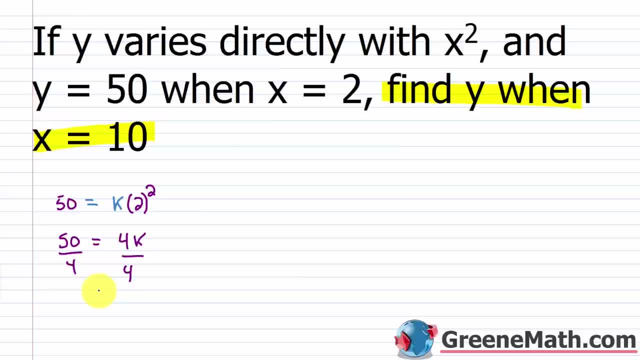 But it is divisible by 2.. 50 divided by 2 is 25.. So what you'd end up with is 25 halves Is equal to k. Let's drag this Up here And we're going to apply that. 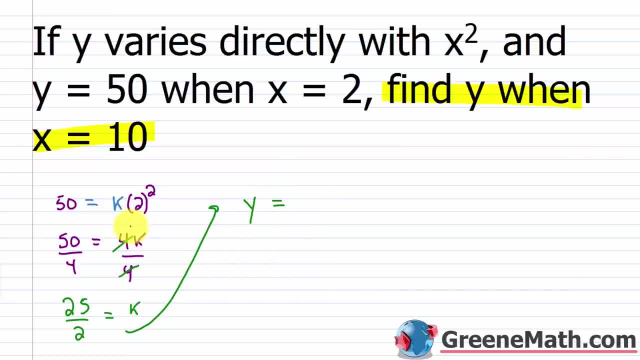 So we want to find y now when x equals 10.. So we don't know what y is. We know that k is 25 halves And we know that x is 10. And we know that it's squared, So 10 squared. 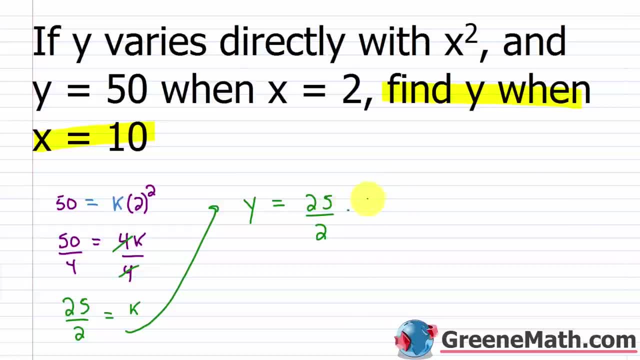 Is 100. So let's go ahead and write that out. So we'd have times 100 here And essentially this is going to cancel with this And give me a 50. And we'd have 50 times 25.. Now to do this easily. 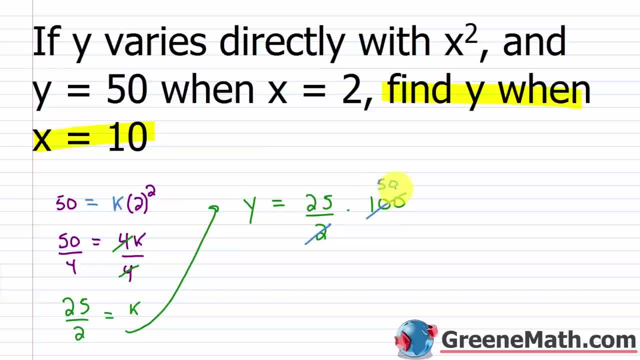 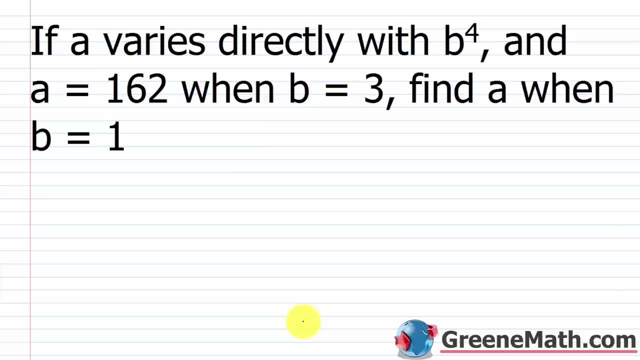 5 times 25 is 125.. Put a 0 at the end, You get y is equal to 1250.. Let's take a look at one more. So if a varies directly with b to the 4th power, 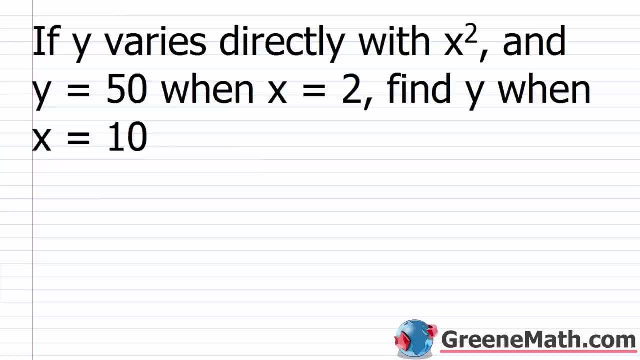 directly with x squared, and y equals 50 when x equals 2, find y when x equals 10. So the equation with direct variation as a power, we just write that y is equal to k times x to the nth power, and we're just going to plug in. It's just that simple. So if y varies directly with x squared, so instead of an n, I'm going to put a 2 there, and then y equals 50. So I'm going to replace 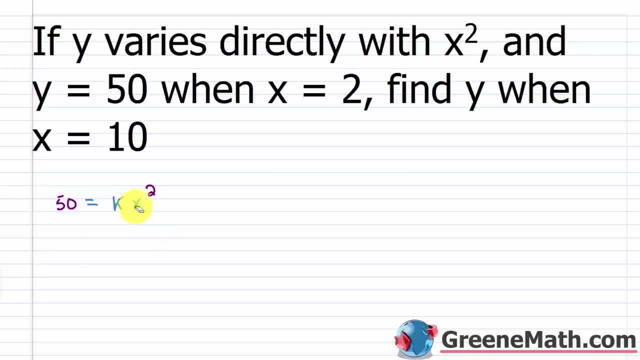 this with a 50 when x equals 2. Find y when x equals 10. So let's find k first, and then we'll deal with this scenario second. Okay, so 2 squared is obviously 4, so you would get 50 is equal to 4k. Divide both sides of the equation by 4, and 50 is not divisible by 4, but it is divisible by 2. 50 divided by 2 is 25, so what you'd end up with is 25 halves is equal to k. Let's drag this up here, and we're going to apply that. So we want to find y now when x equals 10. So we don't know what y is. We know that k is 25 halves. 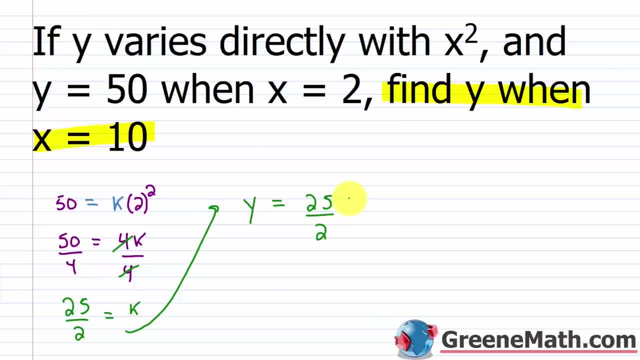 And we know that x is 10, and we know that it's squared. So 10 squared is 100. So let's go ahead and write that out. So we'd have times 100 here, and essentially this is going to cancel with this and give me a 50, and we'd have 50 times 25. Now to do this easily, 5 times 25 is 125. Put a 0 at the end. You get y is equal to 1,200. 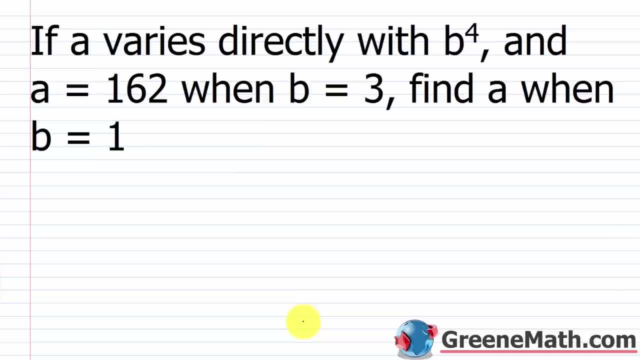 All right, let's take a look at one more. So if a varies directly with b to the 4th power, and a equals 162 when b equals 3, find a when b equals 1. So again, when they kind of throw these different letters at you, just start out with what you know. Don't panic. Just say, okay, well, I know from my formulas that I memorized that y is equal to k times x to the nth power. Okay, so now I have a, that varies directly with b to the 4th power. So a takes the place of y. I still have my k. And then b to the 4th power is going to take the place of x to the nth power. So it's just that simple. Just write what you know, and then just substitute based on the problem. Once you have a general understanding of this, it's going to be very, very easy to do. All right, so the next part is that a equals 162, 162 when b equals 3. 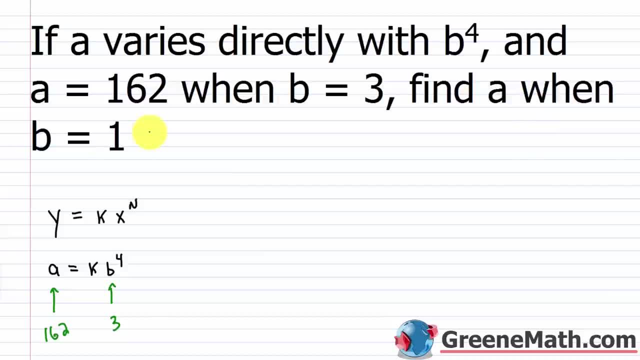 So b is going to be 3. Then find a when b equals 1. So we'll deal with this last. The first thing we want to do is just find k. So let's figure out what that's going to be. Let's drag this up here. So I'd have 162 is equal to 3 to the 4th power, which is what? 3 times 3 is 9. 9 times 3 is 27. 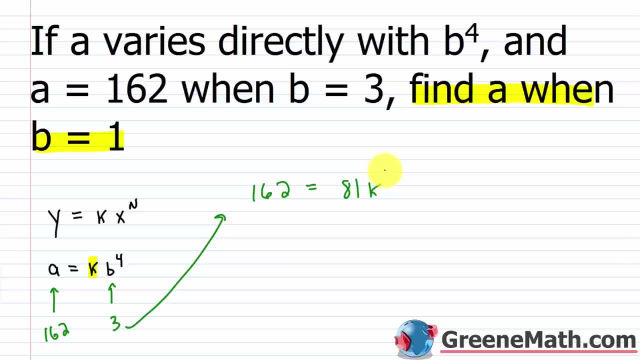 27 times 3 is 81. So this would be 81k. And if I divide both sides of the equation by 81, this is going to cancel with this. 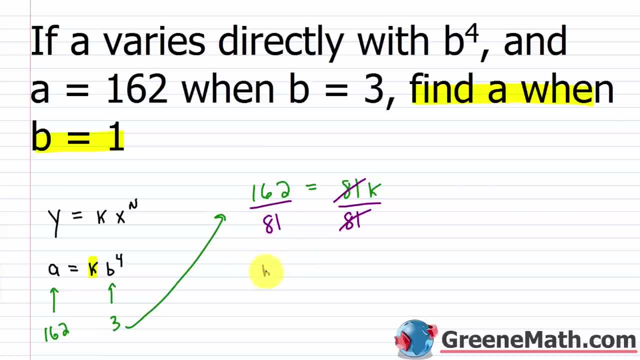 And 162 over 81 is 2. So this is k is equal to 2. Now that I have that information, they want me to find a when b equals 1. So I want a is equal to. I know that k is 2. I'm going to plug in a 2 for that. And I know that b here is 1. So I'd have 1 to the 4th power, which I'm basically just multiplying by 1. So again, as I just said, 1 to the 4th power is 1. 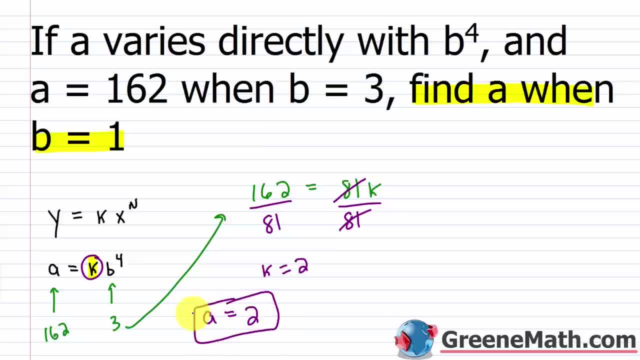 And then 1 times 2 is 2. So a here is going to equal 2. So that's going to be your answer. 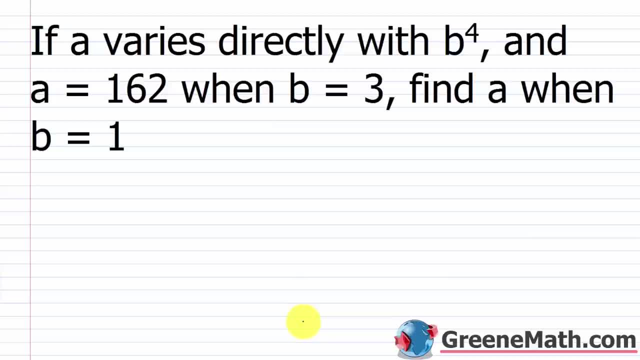 And a equals 162.. When b equals 3.. Find a when b equals 1.. So again, When they kind of throw these different letters at you, Just start out with what you know. Don't panic, Just say, okay, well, I know. 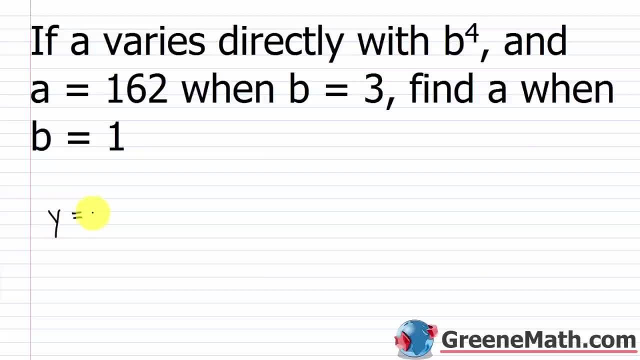 I know the formulas that I've memorized: That y is equal to k times x to the nth power. Okay, So now I have a that varies directly with b to the 4th power. So a takes the place of y. 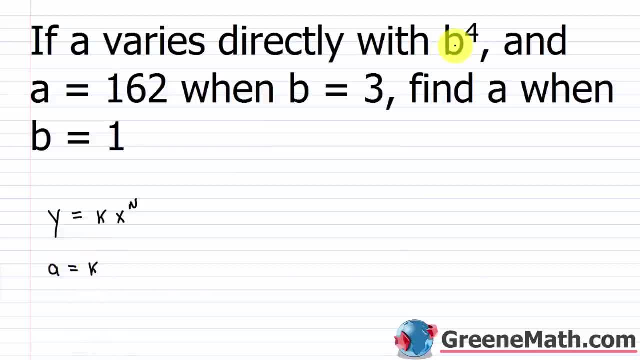 I still have my k And then b to the 4th power Is going to take the place of x to the nth power. So it's just that simple. Just write what you know And then just substitute Based on the problem. 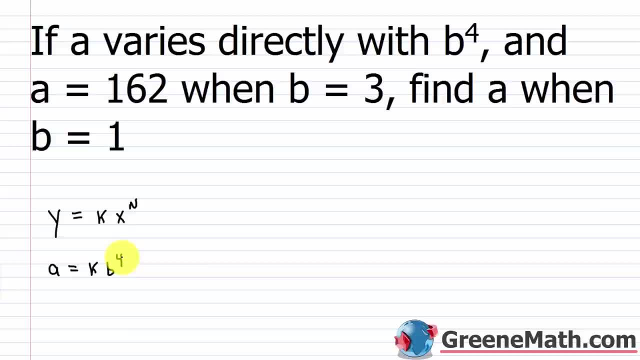 Once you have a general understanding of this, It's very, very easy to do. Alright, so the next part is that a equals 162.. 162. When b equals 3.. So b is going to be 3.. Then find a when b equals 1.. 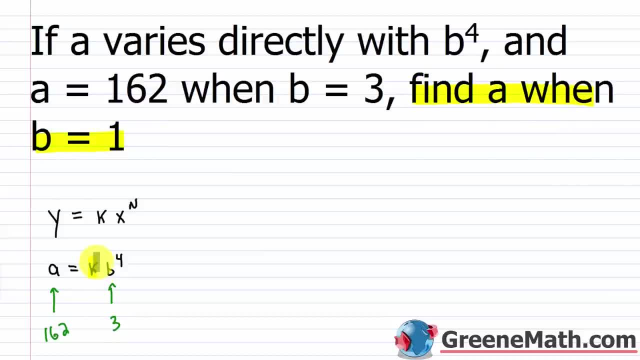 So we'll deal with this last. The first thing we want to do is just find k, So let's figure out what that's going to be. Let's drag this up here. So I'd have: 162 is equal to 3 to the 4th power. 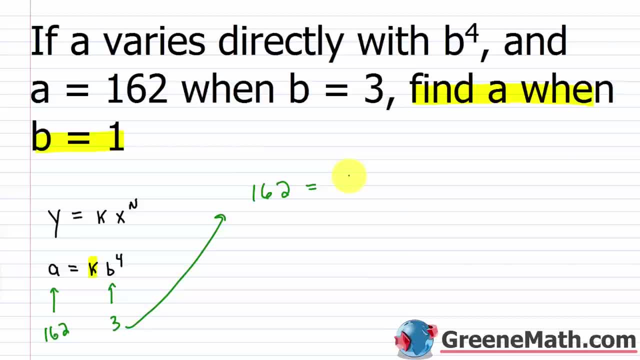 Which is what? 3 times 3 is 9.. 27 times 3 is 81. So this would be 81k, And if I divide both sides of the equation By 81. This is going to cancel with this. 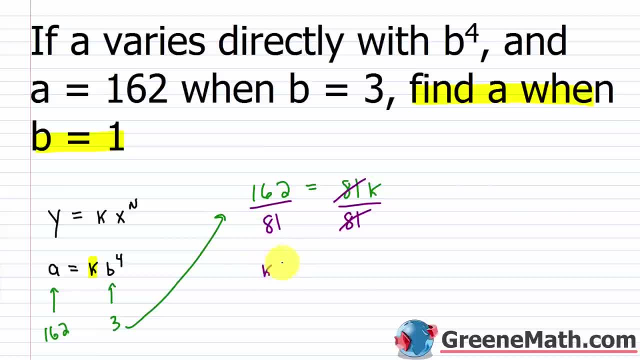 And 162 over 81 is 2.. So this is: k is equal To 2.. Now that I have that information, They want me to find a when b equals 1.. So I want a Is equal to. I know that k is 2.. 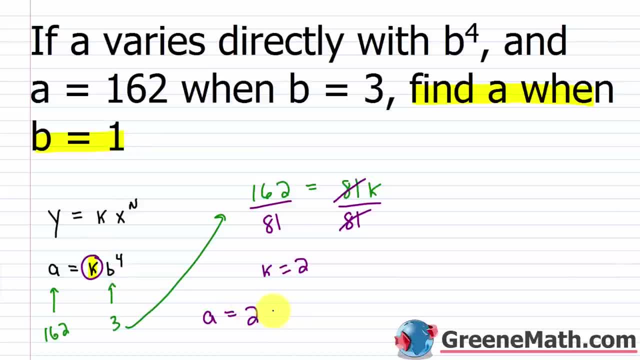 I'm going to plug in a 2 for that. So I'd have 1 to the 4th power, Which I'm basically just multiplying by 1.. So again, as I just said, 1 to the 4th power is 1.. 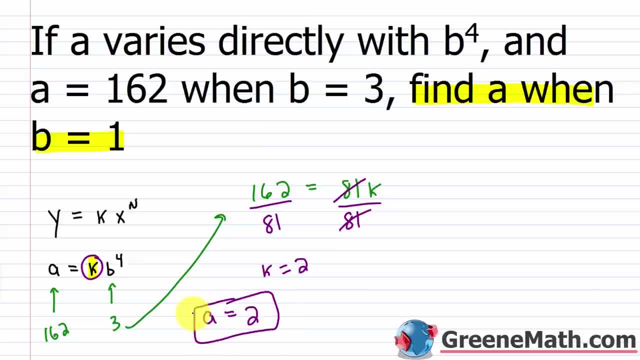 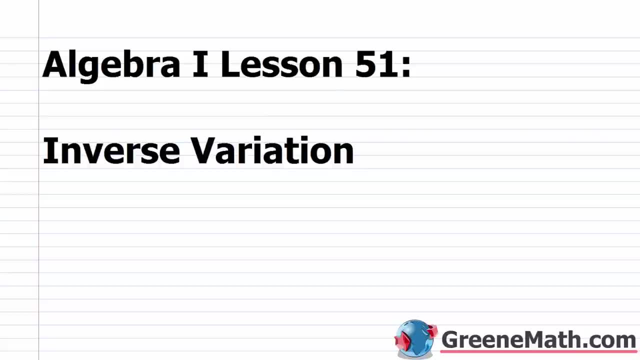 And then 1 times 2 is 2.. So a here is going to equal 2.. That's going to be your answer. Hello and welcome to algebra 1, lesson 51.. In this video we're going to learn about Inverse variation. 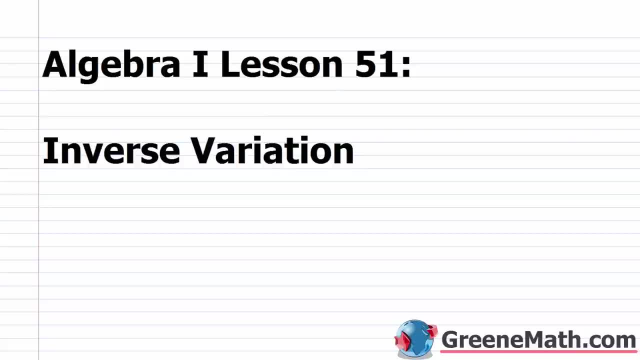 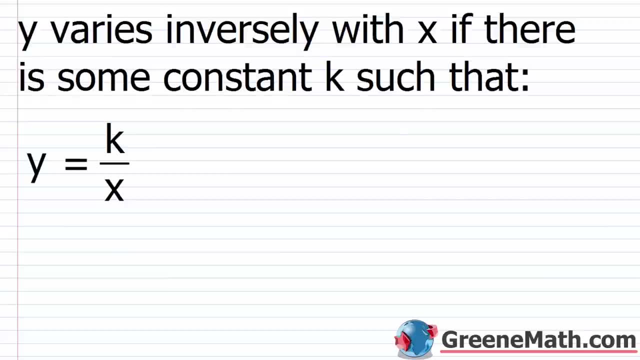 Hello, and welcome to Algebra 1, Lesson 51. In this video, we're going to learn about inverse variation. So in our last lesson, we talked about something known as direct variation. And we saw with that we had y varies directly with x if there is some constant k, such that we had y is equal to k times x, where again, this k is called the constant, the constant of variation. And we talked about a lot of things in that opening lesson. We discussed the fact that in this scenario, if k was positive, so if k was greater than 0, as x increases, y increases. 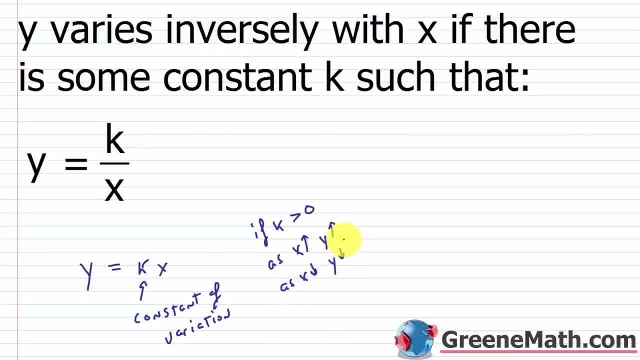 And as x decreases, y decreases. And more specifically, we could say, as x increases by 1 unit, y increases by k units. 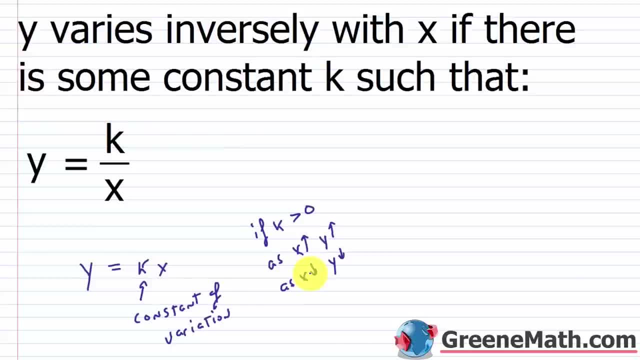 Now we're going to talk about another scenario that you're going to encounter in Algebra 1, and that's called inverse variation. So the concept is the same. So we have that y varies inversely with x if there is some constant k, such that, and here we have y equals k 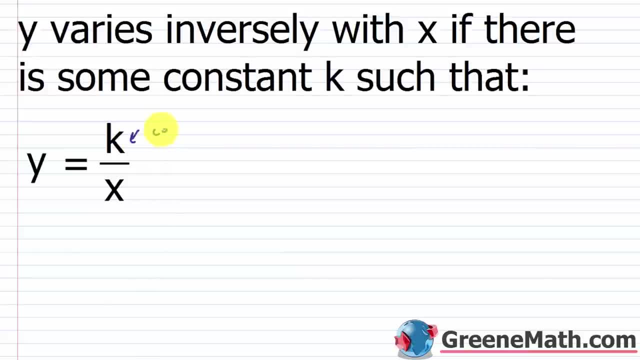 over x. So again, the k is called the constant. The constant of variation. 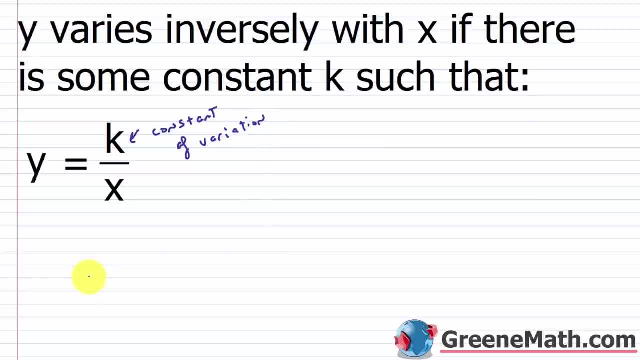 Now what's different here is that if k is greater than 0, now as x increases, what's going to happen to y? Well, just think about this for a second. If x is in the denominator, if x is getting bigger and bigger, what's happening to y? Well, it's getting smaller, right? y is going to decrease. 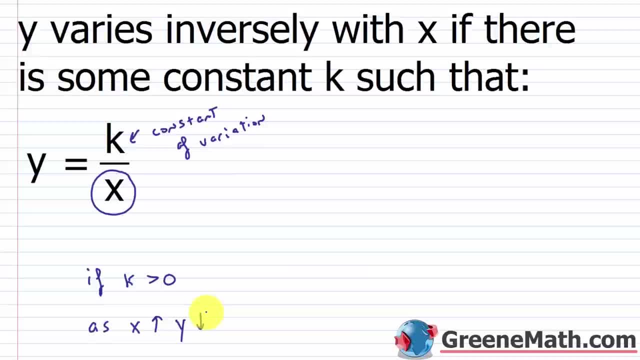 And the thing about this, let's think about some money, for example. Let's say the four of us get together and do a job. So let's say we're getting paid $100 for this job, and we divide it by four 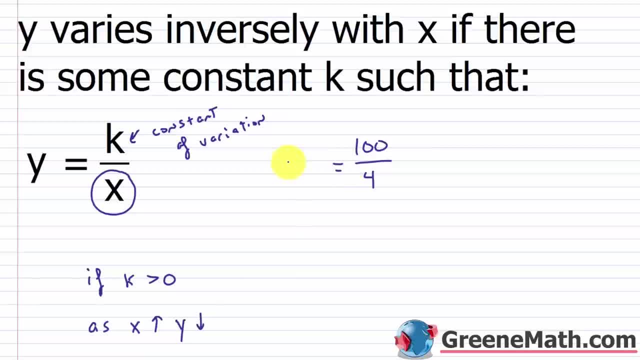 people. And this amount here tells us how much each person is going to get. In this case, that's 25. Now, if I increase the number of people in the group, let's say I take this up to 5. Okay, so x goes up to 5. 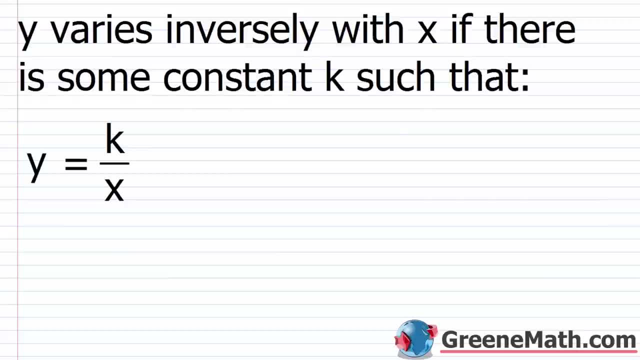 So in our last lesson we talked about something known as Direct variation And we saw with that we had Y varies directly with x If there is some constant k, Such that we had Y is equal to k Times x, Where again this k is called the constant. 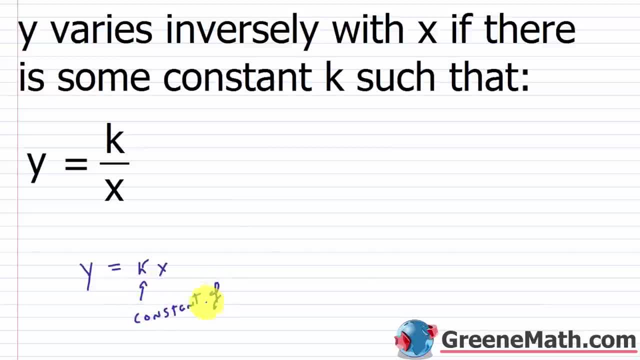 The constant Of Variation. We talked about a lot of Things in that opening lesson. We discussed the fact that in this scenario, If k was positive, So if k was Greater than 0. As x increases, Y increases. 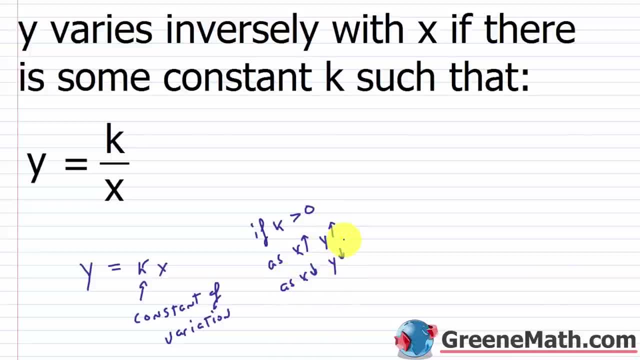 And more specifically, We could say: As x increases by 1 unit, Y increases by K units, Or as x decreases by 1 unit, Y decreases by K units, And so on and so forth. Now we're going to talk about another scenario. 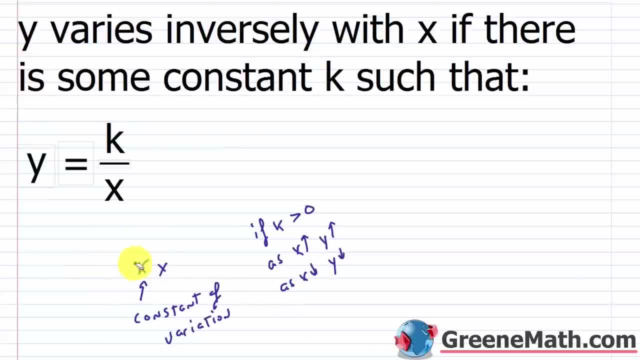 That you're going to encounter in algebra 1.. And that's called inverse variation. So the concept Is the same. So we have that y varies Inversely with x If there is some constant k, Such that, And here we have, y equals k over x. 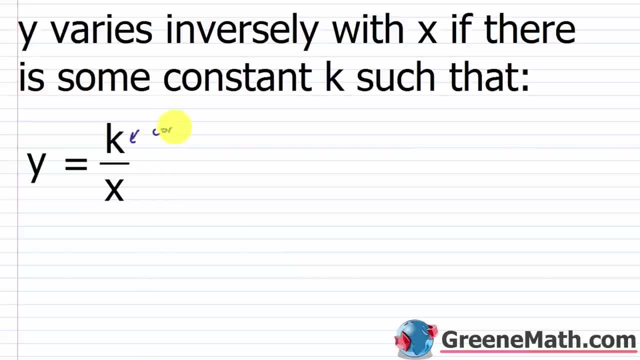 So again, the k Is called the constant, The constant Of variation. Now, what's different here Is that if K is greater than 0. Now, As x Increases, What's going to happen to y? Well, just think about this for a second. 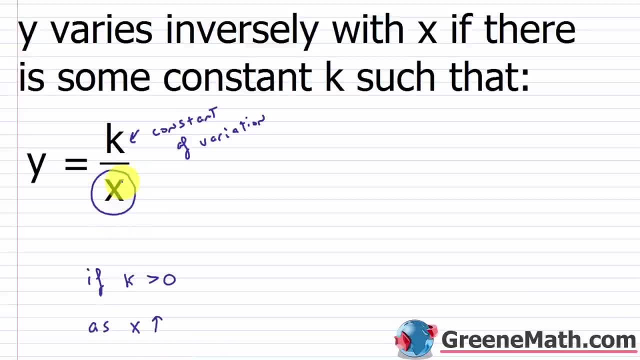 If x is in the denominator, If x is getting bigger and bigger, What's happening to y? Well, it's getting smaller, right, Y is going to decrease. And the thing about this? Let's think about some money, for example, Let's say the 4 of us. 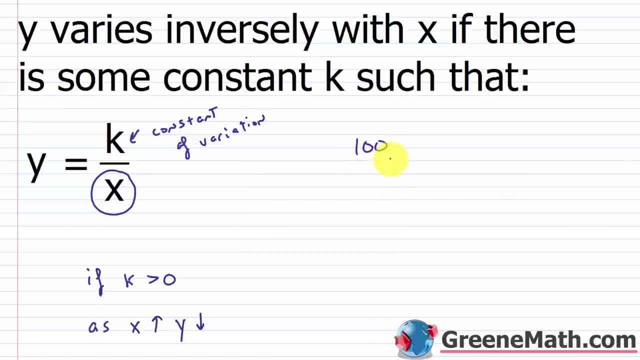 Get together and do a job. So let's say We're getting paid $100 for this job And we divide it by 4 people And the number here tells us How much each person is going to get. In this case that's 25.. 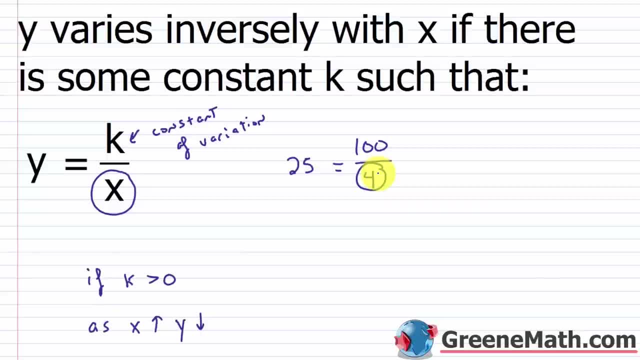 Now, if I increase the number of people in the group, Let's say I take this up to 5.. Okay, so x goes up To 5.. What's going to happen to y? Well, it's going to go down. It's going to go to 20.. 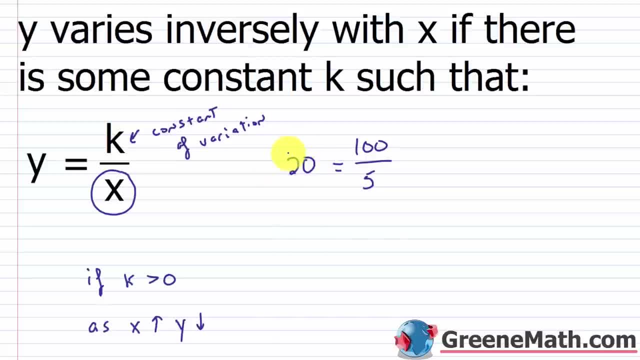 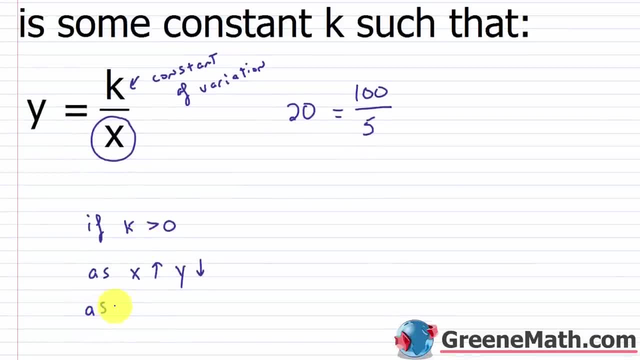 So as I divide by a larger number, I am getting a smaller result, And again, this is when k is a positive Value. But the opposite is also true. As x decreases, Y increases, Right. so if I take this From 5 to, let's say, 2.. 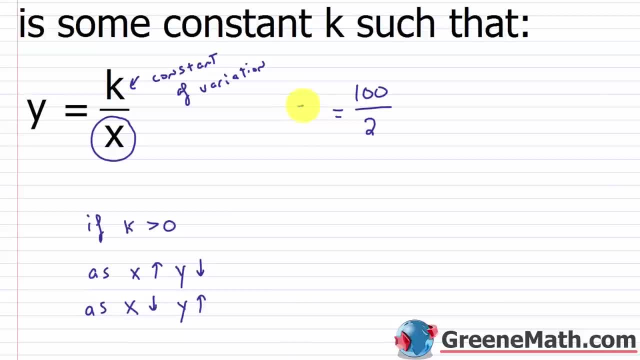 Now, 100 divided by 2 is 50. So that's going to increase. So again, As x goes down, Y goes up, And as x goes up, Y goes down. So this is the opposite of what we saw With direct variation. 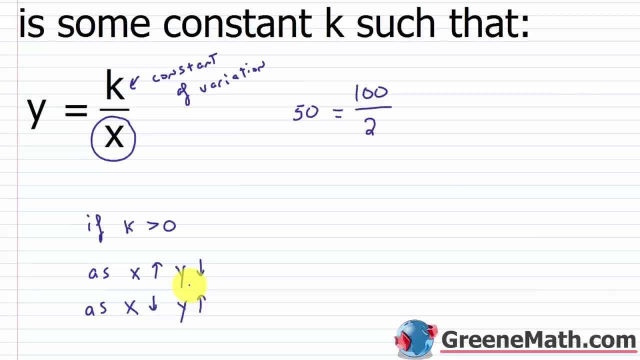 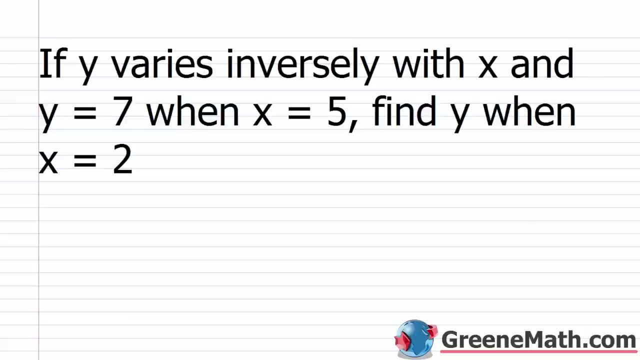 Where, as x went up, Y went up, And that is positive. Alright, so let's jump in and just look at a typical problem. You solve these problems the same way That you approach them with direct variation. So we have: If y varies inversely with x, 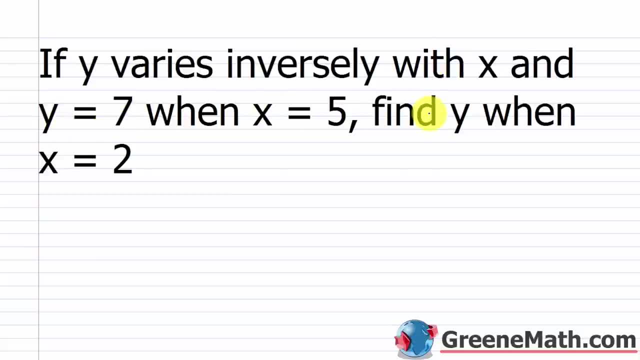 And y equals 7.. When x equals 5. Find y when x equals 2. So just write your formula So y equals k over x, And just plug in With the information they give you, So we have that y equals 7.. 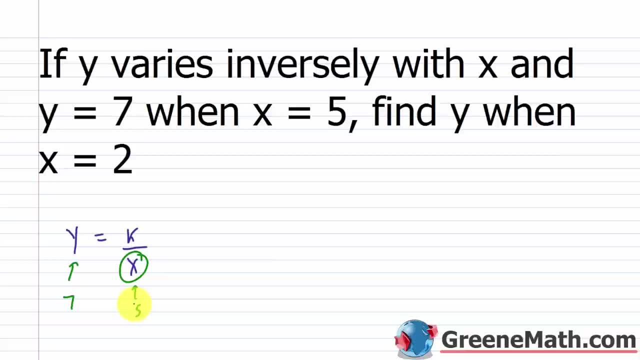 And x equals 5.. Now The shortcut here is to realize that With this generic formula I can multiply both sides of the equation by x, And what I'm going to have is xy is equal to k. So that's kind of what most teachers will teach you as a shortcut. 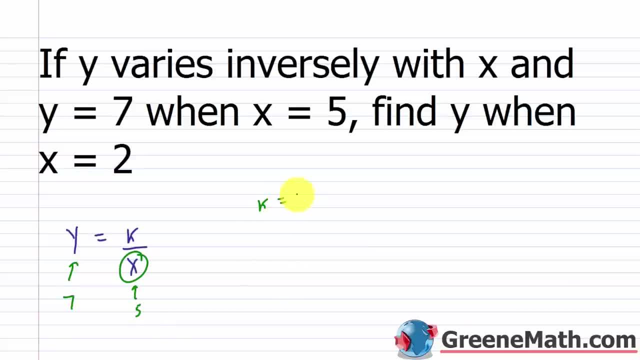 To say: okay, If I want to find k, It's just equal to x times y. So if I plug in A 7 for y And I plug in a 5 for x, I know that k is 35. But this will be 35.. 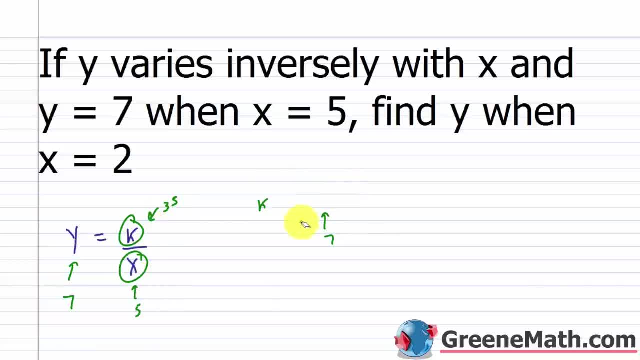 35 divided by 5 is in fact 7.. Okay, So once I know what the value is for k, I can go through And figure out this scenario: Find y when x equals 2.. Well, again I know That k is 35.. 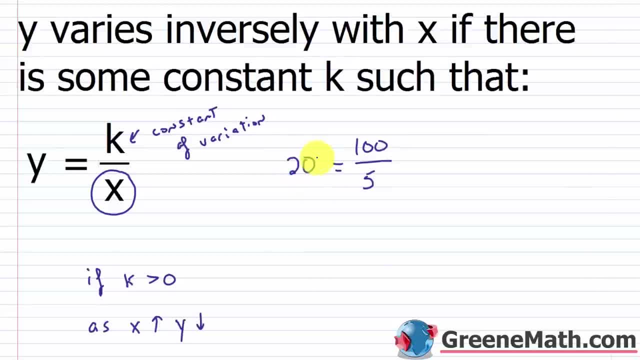 What is going to happen to y? Well, it's going to go down. It's going to go to 20. So as I divide it by a larger number, I am getting a smaller result. And again, this 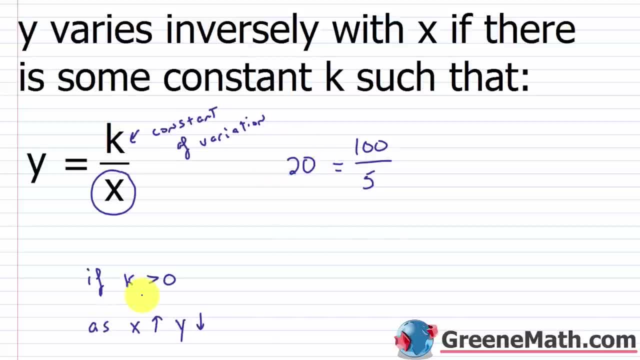 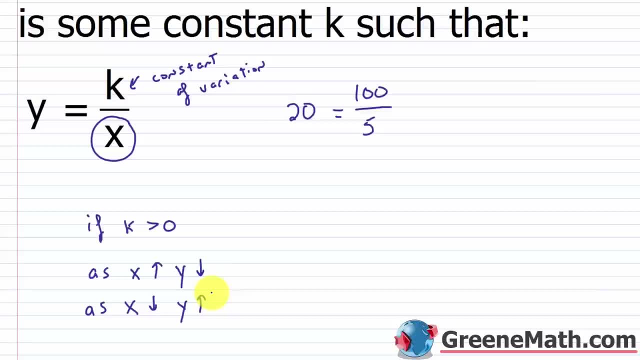 is when k is a positive value. But the opposite is also true. As x decreases, y increases. 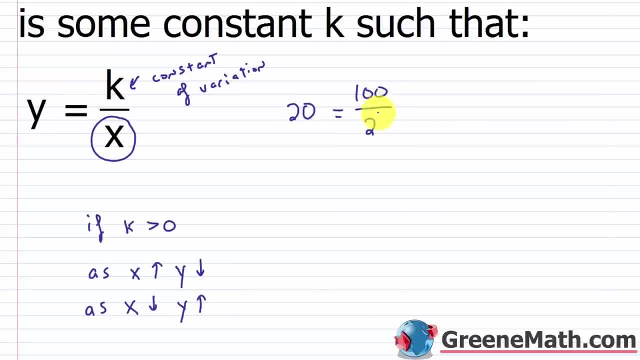 So if I take this from 5 to 2, let's say? Now 100 x 2 is 50, so that's going to increase. So if I take this from 5 to 2, let's say lambda, let's say 1 over 10. Let's say X is 20 times 3 over 5 is great. That's also true. And so as I keeptake the numbers, from 24 times kill, 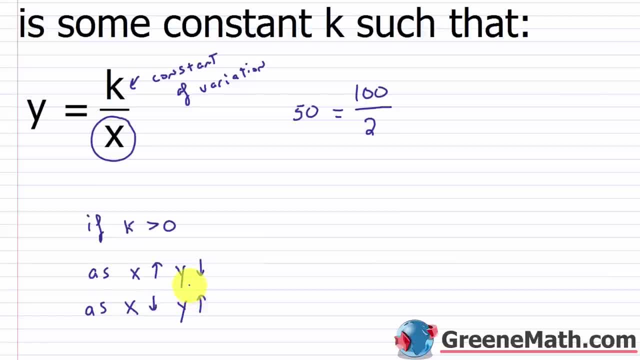 So again, as x goes down, y goes up, and as x goes up, y goes down. 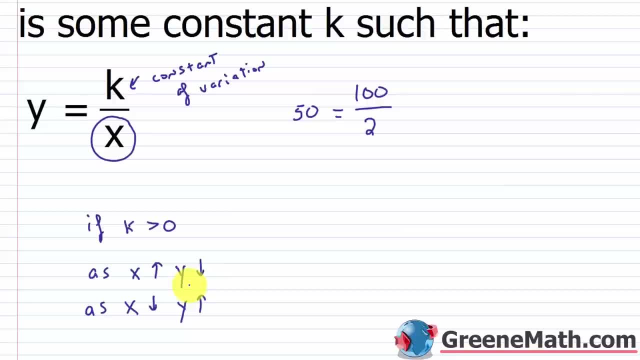 So this is the opposite of what we saw with direct variation, where as x went up, y went up, and as x went down, y went down, again, when k is positive. 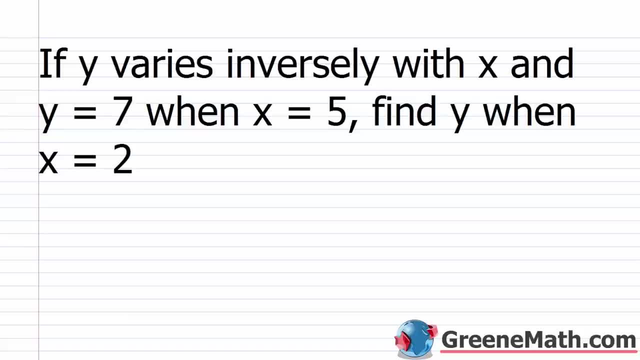 All right, so let's jump in and just look at a typical problem. You solve these problems the same way that you approach them with direct variation. 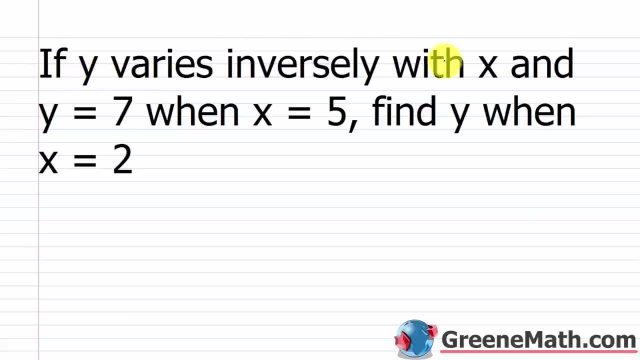 So we have if y varies inversely with x, and y equals 7 when x equals 5, find y when x equals 2. 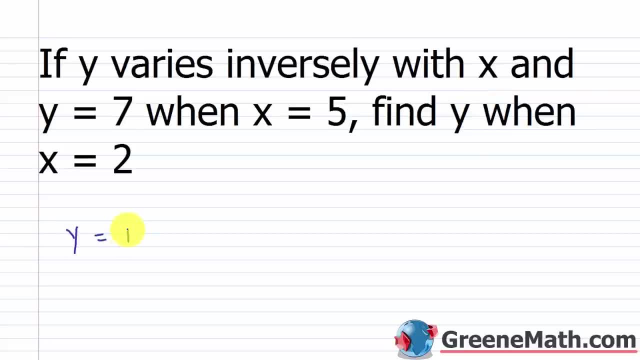 So just write your formula, so y equals k over x, and just plug in with the information they give you. So we have that y equals 7, we have that x equals 5. 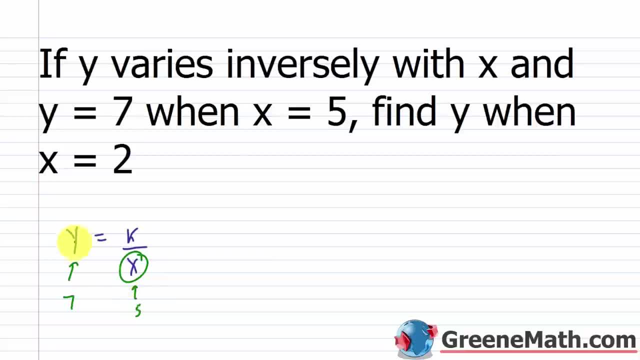 Now, the shortcut here is to realize that with this generic formula, I can multiply both sides of the... 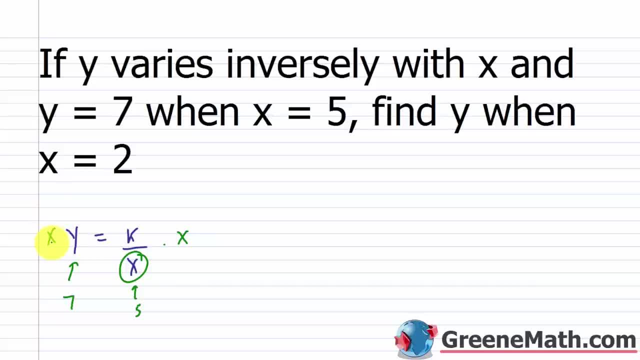 equation by x, and what I'm going to have is x, y is equal to k. 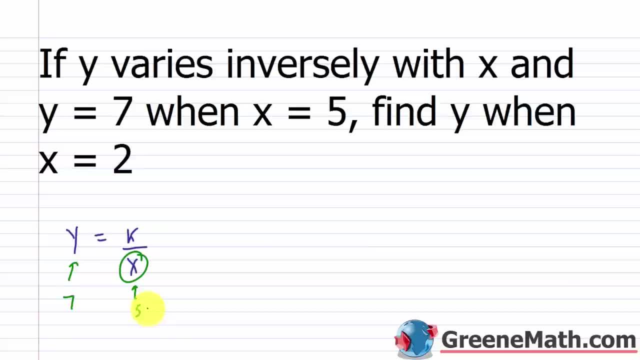 So that's kind of what most teachers will teach you as a shortcut to say, okay, if I want to find k, it's just equal to x times y. 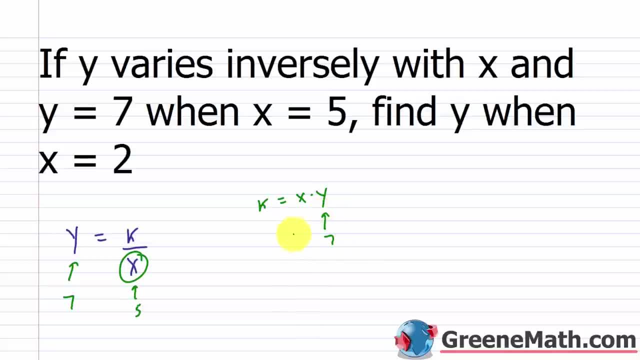 So if I plug in a 7 for y, and I plug in a 5 for x, I know that k is 35, right? I know that this will be 35. 35 divided by 5 is, in fact, 7. 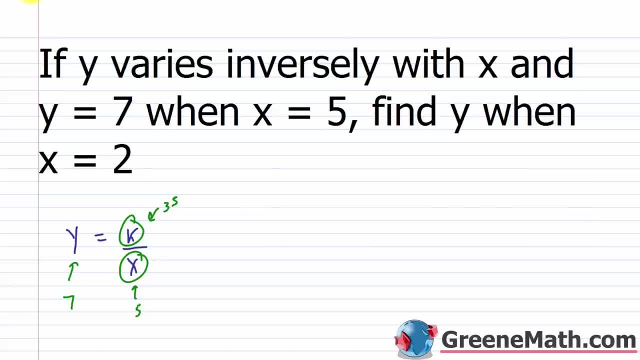 Okay, so once I know what the value is for k, I can go through and figure out this scenario. Find y when x equals 2. 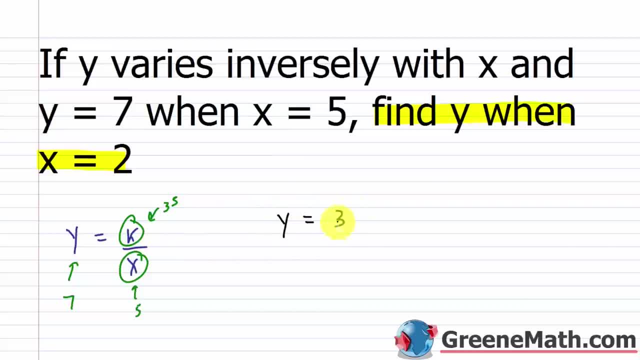 Well, again, I know that k is 35, and x is going to be 2. So I would get 35 halves, which you could write as 17.5 if you wanted to, or you could just keep it in fractional form as 35 halves. All right, let's take a look at the next one. 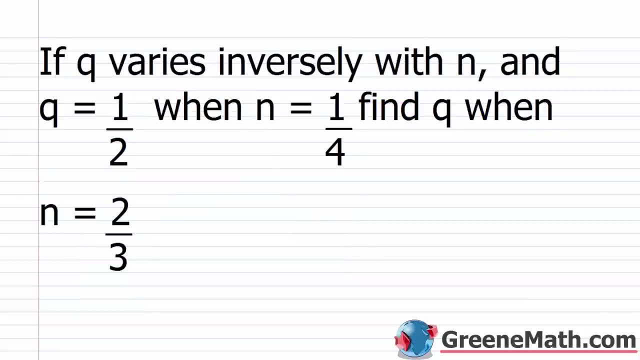 So if q varies inversely with n, and q equals 1 half when n equals 1 fourth, find q when n equals 2 thirds. 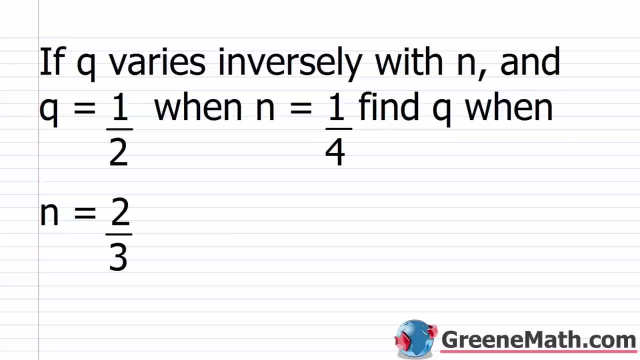 So again, this might be the type of problem that really throws you for a loop, right? You see this, and you're like, oh, I'm used to working with y and x. Just think about what you normally get. Normally, you get if y varies inversely with x, right? 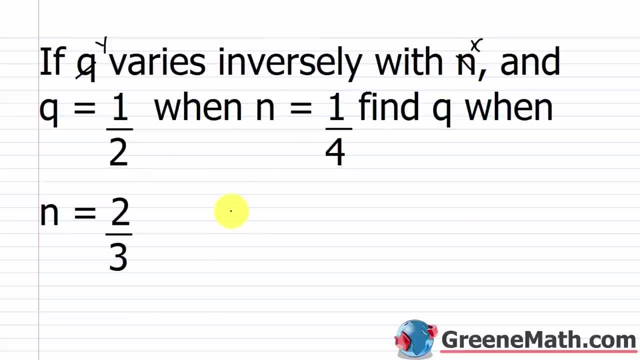 So we would write our equation to start as q is equal to k over n. And once I have that set up, I could just plug in a 7 for y, and I could just keep it in fractional form. So I could just plug in and get my answer. 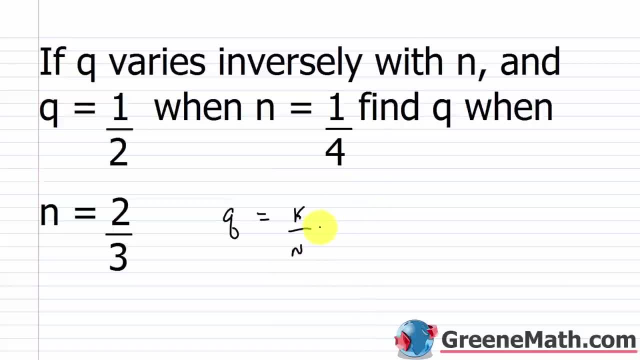 Now, we know that to find k, we can multiply both sides by n. So I can multiply this by n, multiply this by n, and I could say k is equal to what? n times q. 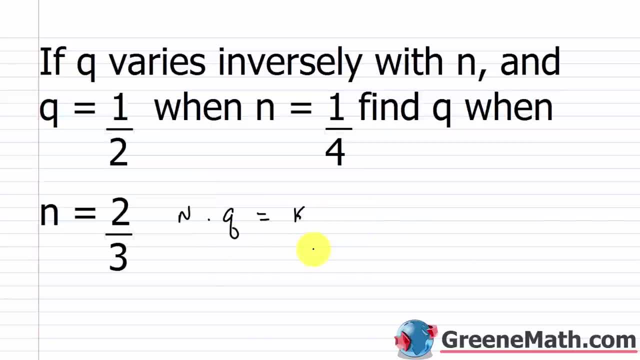 So in the first scenario, the scenario they give us so that we can find k, we're told that q is 1 half. So q is 1 half. And we're told that n is 1 fourth. So n is 1 fourth. And so 1 fourth times 1 half would be 1. So k is equal to 1 eighth. Okay. 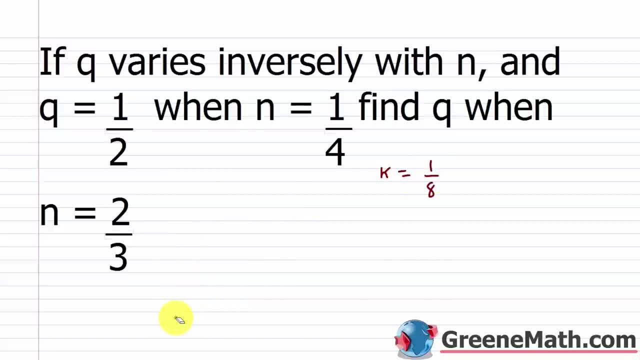 So now that we know that, we're told to find q when n equals 2 thirds. So we have q is equal to, we'll have 1 eighth, 1 eighth, divided by 2 thirds. So what we're going to do here, we're going to have q is equal to 1 eighth times the reciprocal of 2 thirds, which is 3 halves. This is going to be equal. This is going to be equal to 3 over 16. So q in this scenario is going to be 3 sixteenths. Okay. 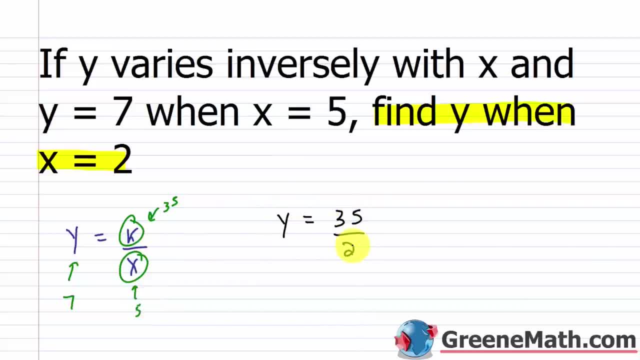 And x is going to be 2.. So I would get 35 halves, Which you could write as 17.5.. If you wanted to, Or you could just keep it in fractional form As 35 halves. Alright, let's take a look at the next one. 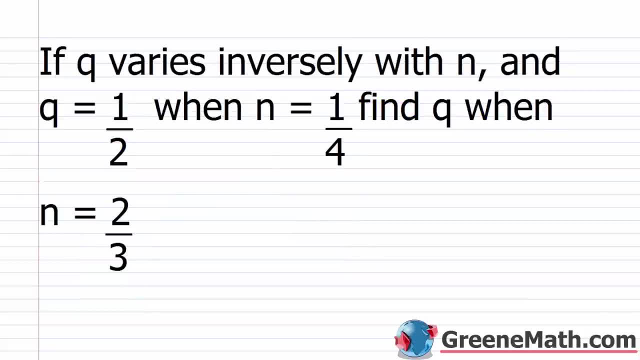 So if q varies inversely with n And q equals 1 half When n equals 1 fourth, Find q when n equals 2 thirds. So again, This might be the type of problem That really throws you for a loop. 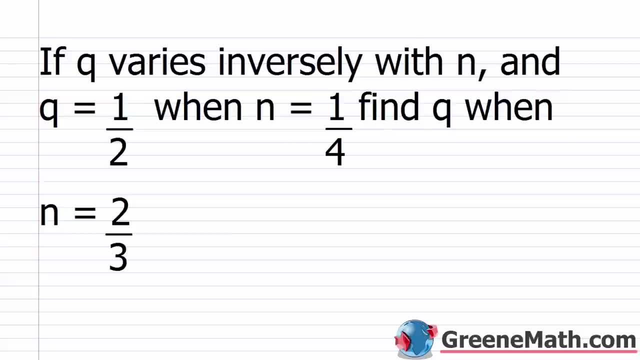 You see this and you're like: I'm used to working with y and x. Just think about what you normally get. Normally you get, if y varies inversely with x, Right, So we can write our equation to start, as q is equal to. 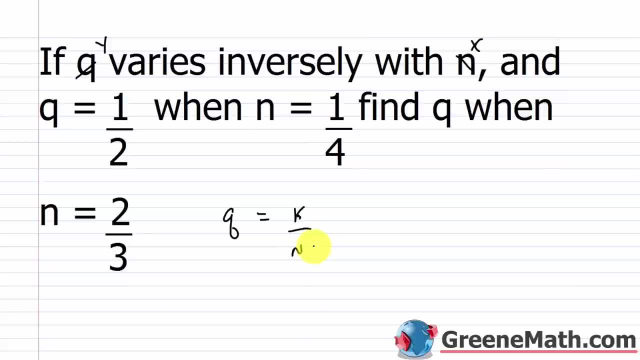 k over n And once I have that set up, I can just plug in and get my answer. Now we know that To find k We can multiply both sides by n, So I can multiply this by n. Multiply this by n. 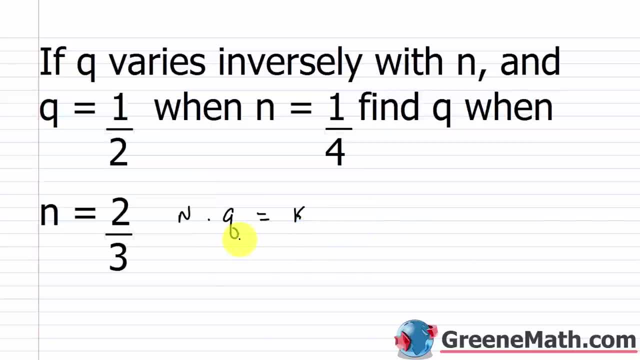 And I can say k is equal to what n times q. So in the first scenario, The scenario they give us so that we can find k, We're told that q is 1 half, So q is 1 half, And we're told that n is 1. fourth, 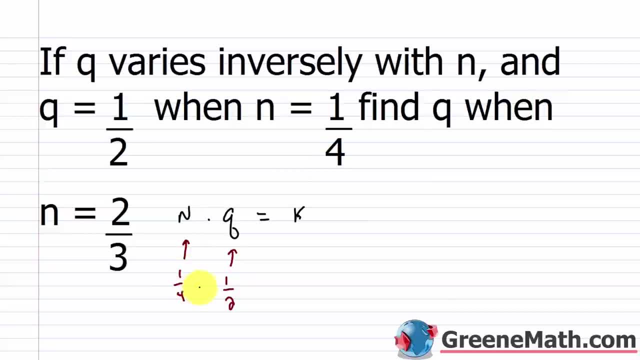 So n is 1 fourth, And so 1 fourth times 1 half would be 1 eighth. So k is equal to 1 eighth. So now that we know that We're told to find q When n equals 2 thirds, 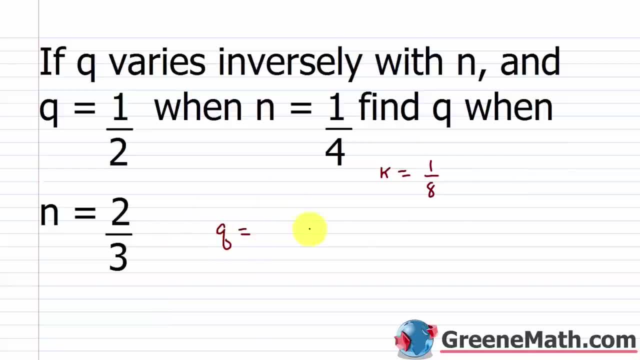 So we have q is equal to: We'll have 1 eighth Divided by 2 thirds. So what we're going to do here, We're going to have q is equal to 1 eighth Times the reciprocal of 2 thirds. 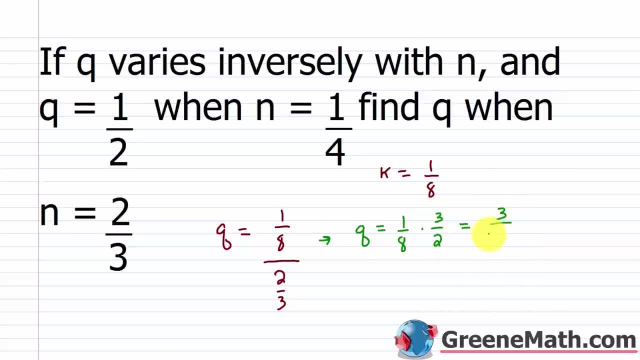 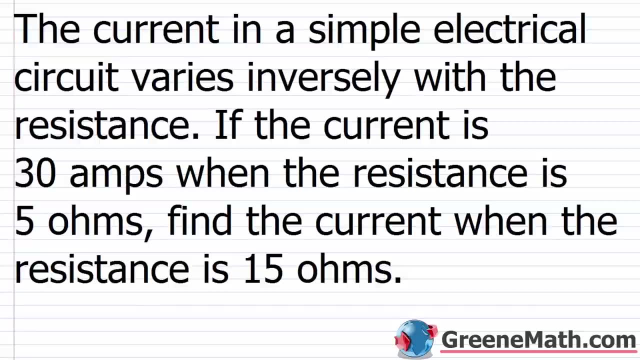 Which is 3 halves. This is going to be equal to 3 over 16.. So q in this scenario Is going to be 3 sixteenths. Okay, let's take a look at a pretty simple word problem That deals with Ohm's law. 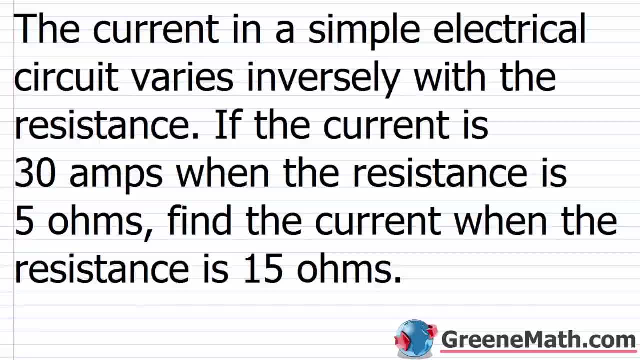 Let's take a look at a pretty simple word problem that deals with Ohm's Law. So this is something that, you know, as an Algebra 1 student, you might have come across this in your science class. You might not have. 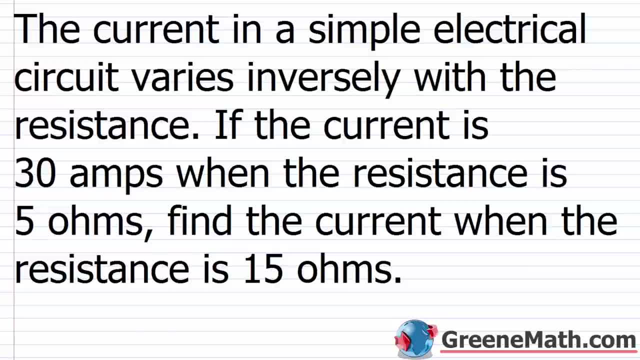 For sure, by the time you get out of high school, you'll be very familiar with this Ohm's Law. 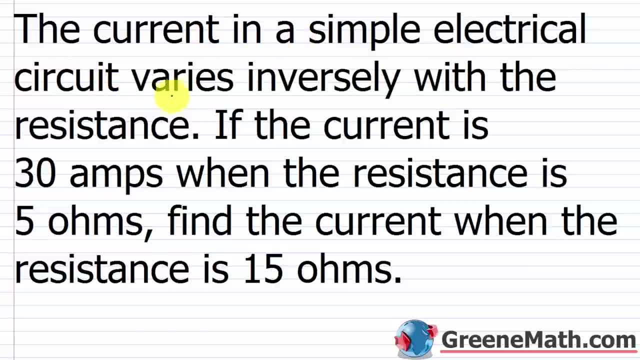 So the current in a simple electrical circuit, varies inversely with the resistance. 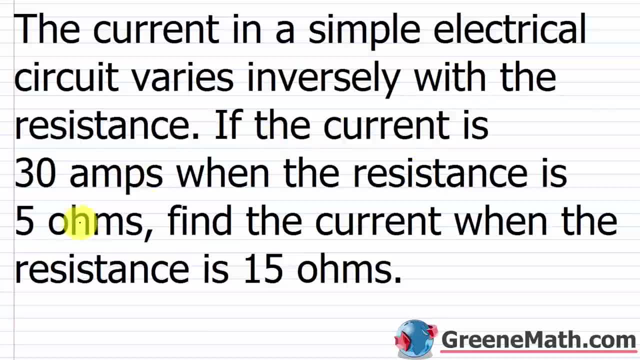 If the current is 30 amps when the resistance is 5 ohms, find the current when the resistance is 15 ohms. 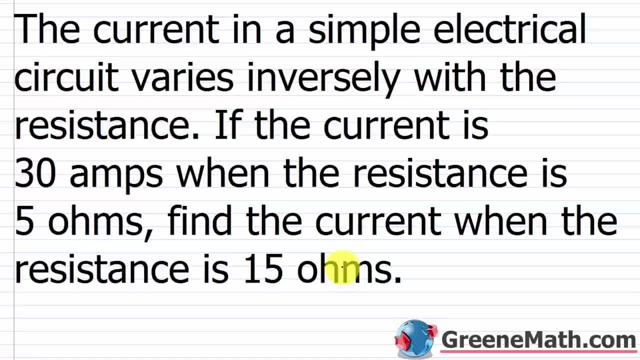 So pretty simple to solve one of these. I'm just going to give you, let me go down to another sheet of paper. 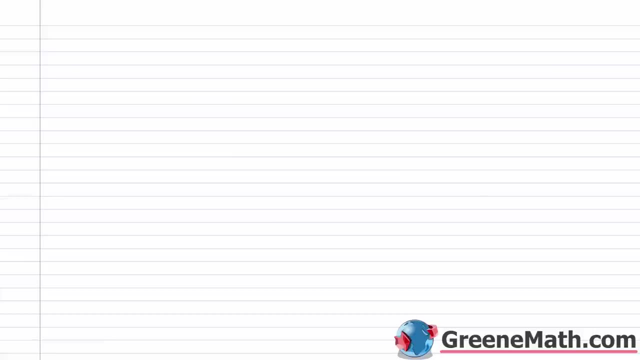 I'm just going to give you the generic notation they use when you talk about Ohm's Law. So Ohm's, Ohm's Law. 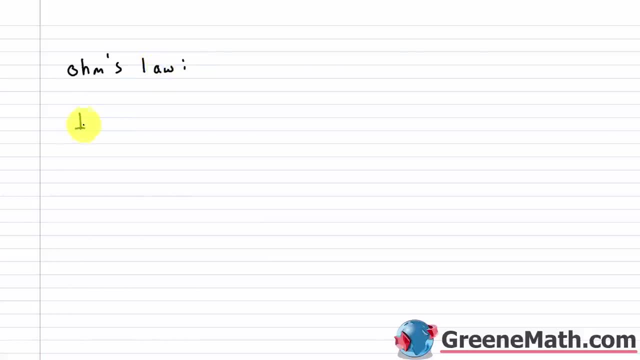 So you have the current. Okay. The current, which is represented with I. So this is for the current. 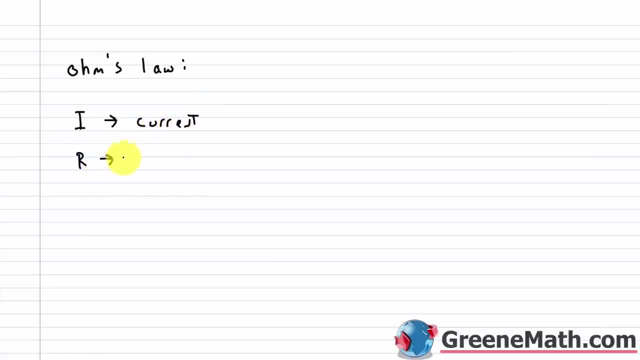 Then you have the resistance, which is represented with R. And then you have the voltage. Now in our word problem, we didn't say anything about voltage, but the voltage is going to be your constant of variation. It's not going to change. 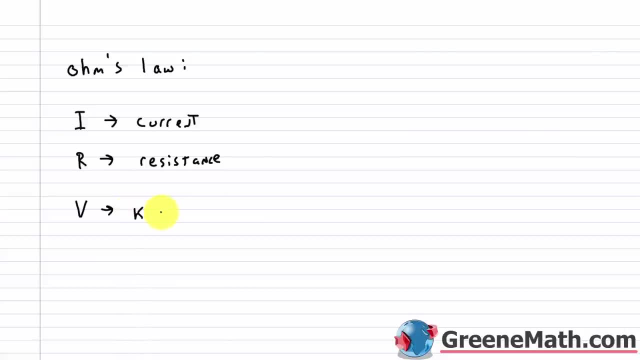 So this is my K or my constant of variation. And it represents the voltage. Okay. 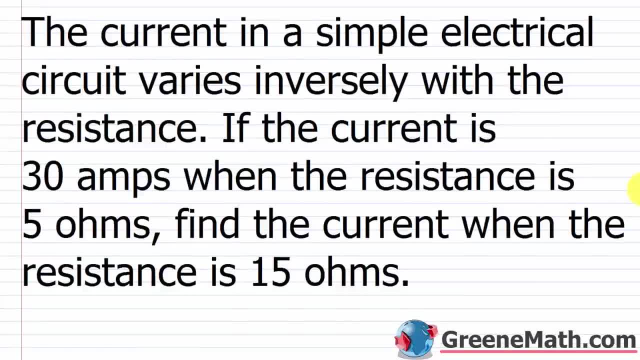 So let's go back up real quick and let's get some numbers going. 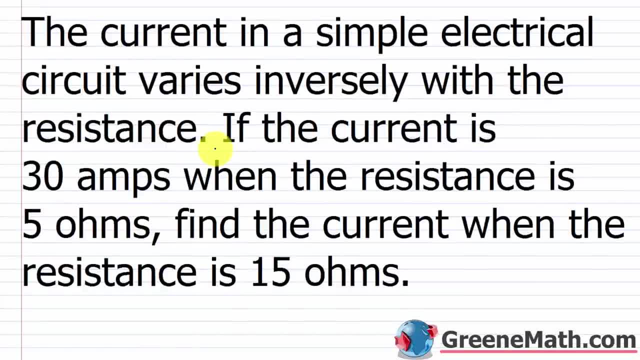 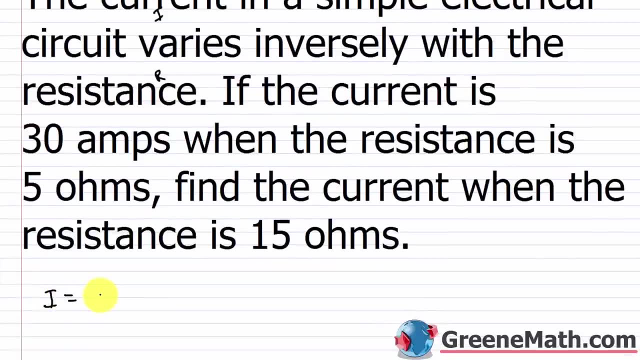 So it says, first off, the current in a simple electrical circuit varies inversely with the resistance. So current we represented with R. And so it means our resistance we represented with R. So that means that our formula would look like this. I is equal to some constant over R. Now we already said that the constant would be V the voltage. So you could put V there, you can put K there. You could really put whatever you want there. It doesn't matter. Right? You're just solving for that unknown. 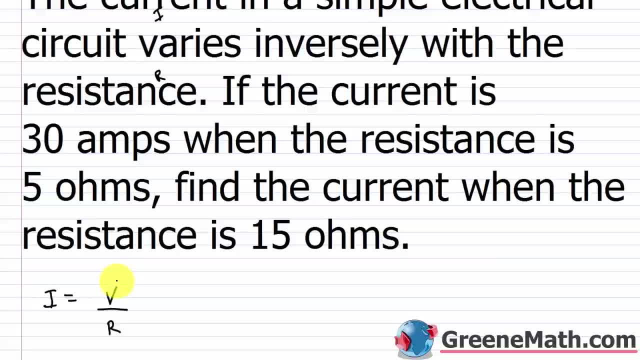 So let's put V there to make sure that we're consistent with that formula. Alright. So it tells us in the starting scenario, if the current is going to be a constant over the voltage, 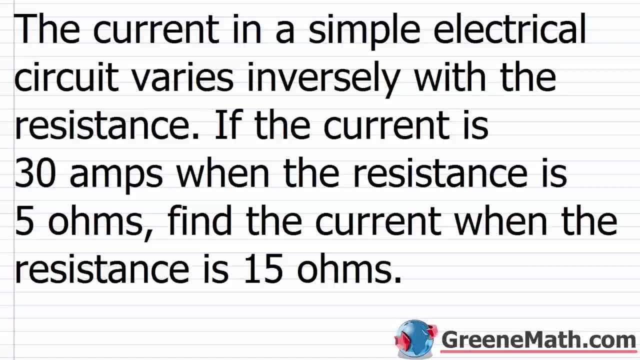 So this is something that You know. as an algebra 1 student, You might have come across this in your Science class. For sure, by the time you get out of high school, You'll be very familiar With this Ohm's law. 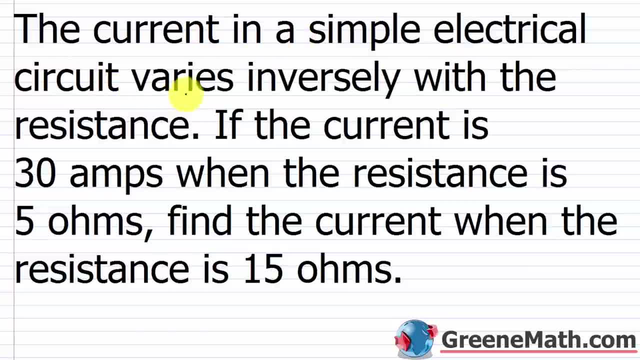 So the current In a simple electrical circuit Varies inversely With the resistance. If the current is 30 amps When the resistance is 5 ohms, Find the current when the resistance Is 15 ohms. So pretty simple to solve one of these. 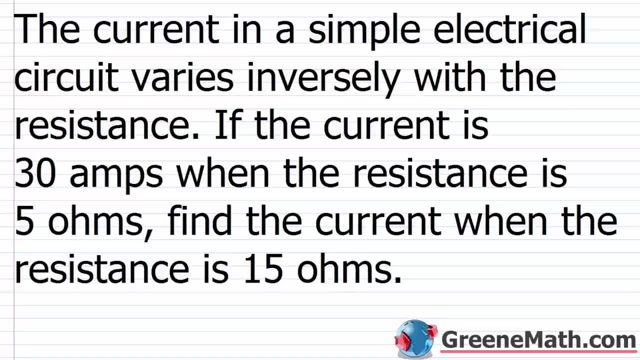 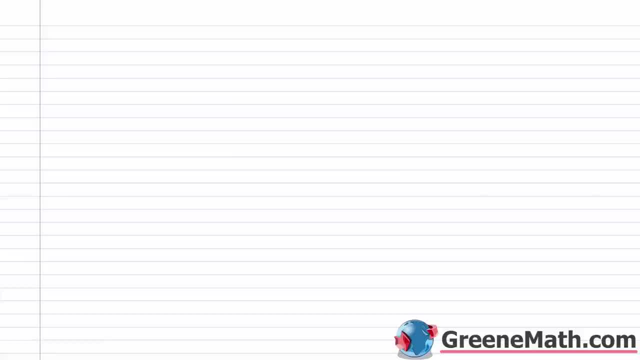 I'm just going to give you. Let me go down to another sheet of paper. I'm just going to give you The generic notation they use When you talk about Ohm's law. So Ohm's, Ohm's law. 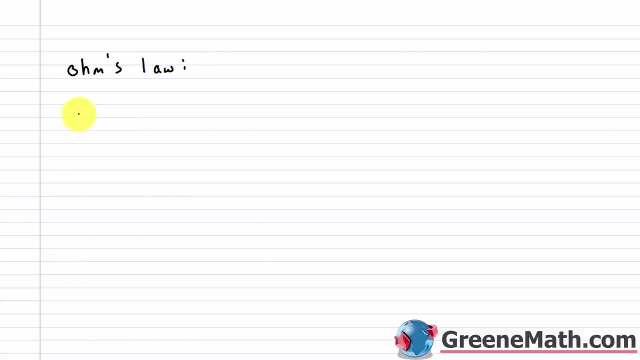 So you have the current- Okay, the current- Which is represented with I. So this is for the current. Then you have the resistance, Which is represented with R, And then you have the voltage. Now, in our word problem We didn't say anything about voltage. 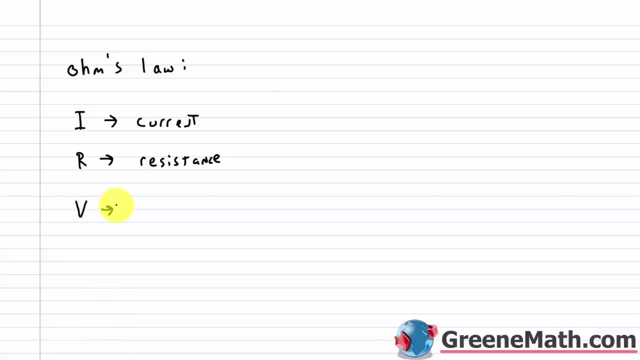 But the voltage is going to be Your constant of variation. It's not going to change. So this is my K, Or my constant Of variation, And it represents The voltage. Okay, So let's go back up Real quick. 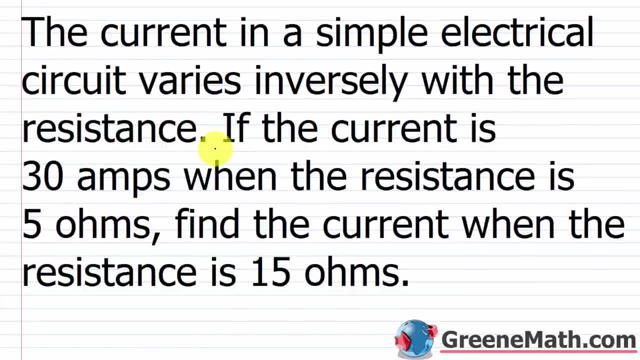 And let's get some numbers going. Because, first off, The current in a simple electrical circuit Varies inversely with the resistance. So current we represented with I, Resistance we represented with R. So that means That our formula would look like this: 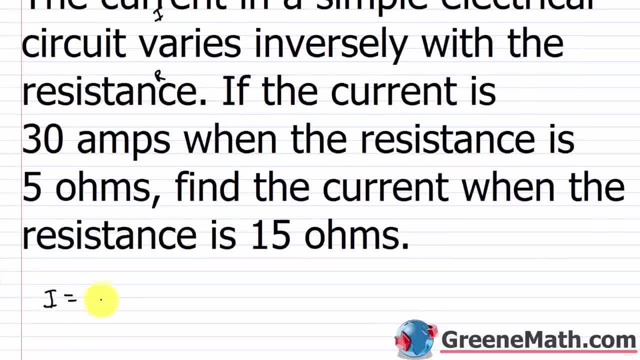 I is equal to Some constant Over R. Now we already said that the constant Would be V, the voltage. So you could put V there, You could put K there, You could really put whatever you want there. So let's put V there. 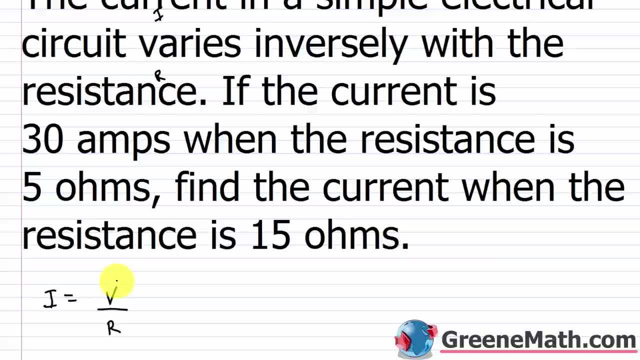 To make sure that we're consistent with that formula. Alright, so it tells us In the starting scenario, If the current is 30 amps. So this is where my current goes, So this would be a 30. When the resistance is 5 ohms. 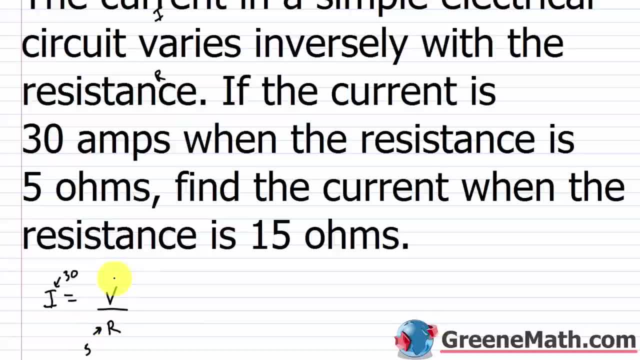 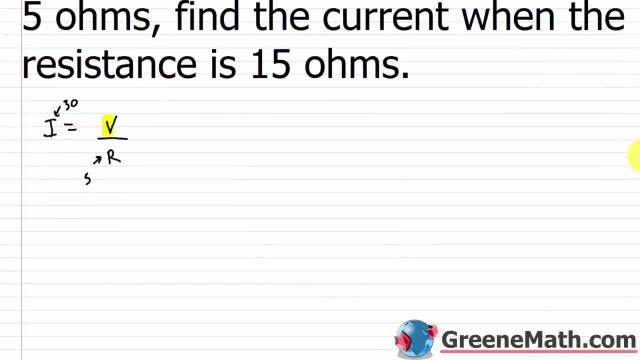 So this would be a 5. And then we'll stop there. We just want to find V And then apply it to that second scenario. So let's solve for that. So what I would do here: I would multiply, We'd have 30.. 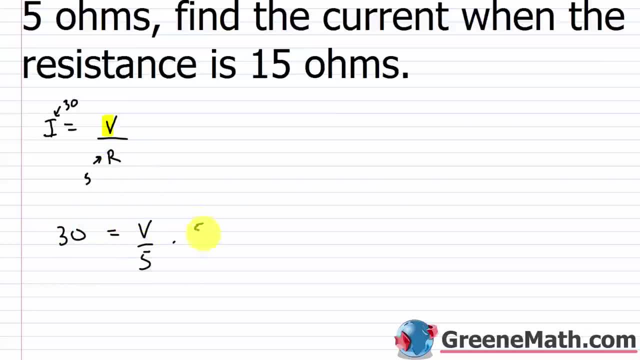 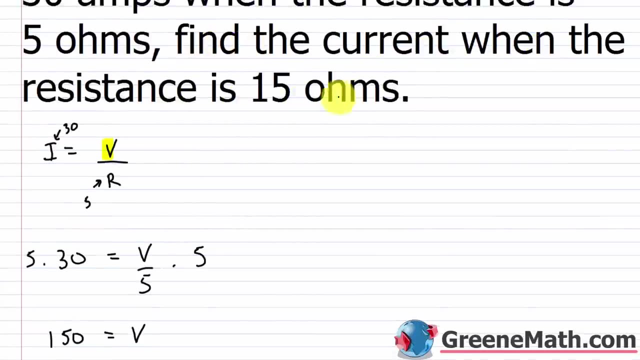 Equals V over 5.. Multiply both sides of the equation By 5. And I would get 150.. Is equal to V. So that's my voltage. That's going to stay the same. So now, in the next scenario, We want to find the current. 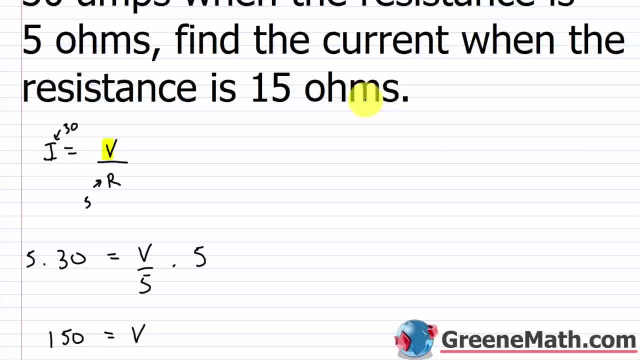 When the resistance is 15 ohms. Now the resistance goes up. That means that the current Is going to go down. So we're looking for a smaller value Than 30 here. So if I plug in I have, I is equal to. 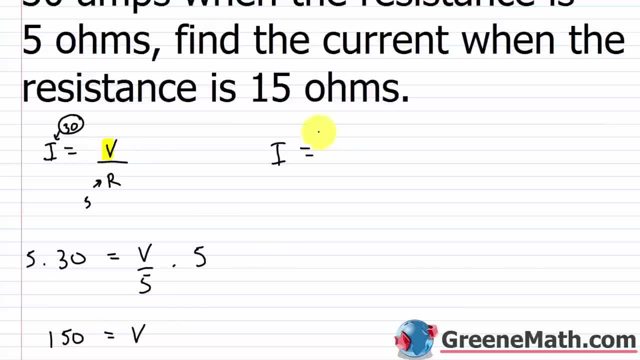 I know that my voltage, Which is V, That's on top, is 150.. And they're giving me this 15.. For the resistance, Pretty easy to do this here: 150 divided by 15 is 10.. So I is equal to 10.. 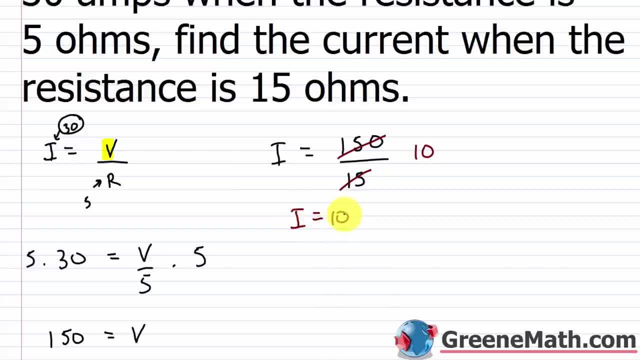 In this scenario, Because it's a word problem, We probably want to Say that the current Is 10 amps When the resistance Is 15 ohms. Okay, One of the things you can notice about this, Again, it's inverse variation. 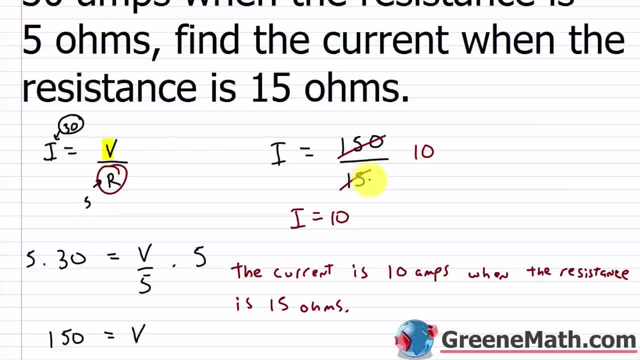 So as R increased, It went from 5 to 15.. The I, or the current, decreased, It went from 30 to 10.. So that's consistent With what we know about inverse variation. Alright, so to kind of wrap up the lesson. 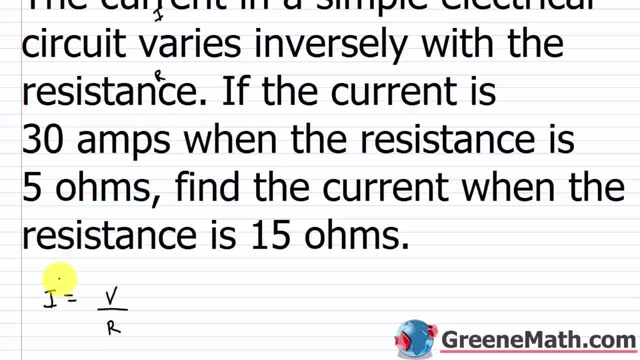 If the current is 30 amps, so this is where my current goes, so this would be a 30. 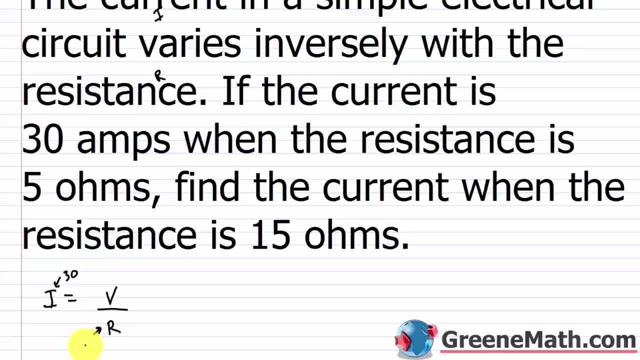 When the resistance is 5 ohms, so this would be a 5. And then we'll stop there. 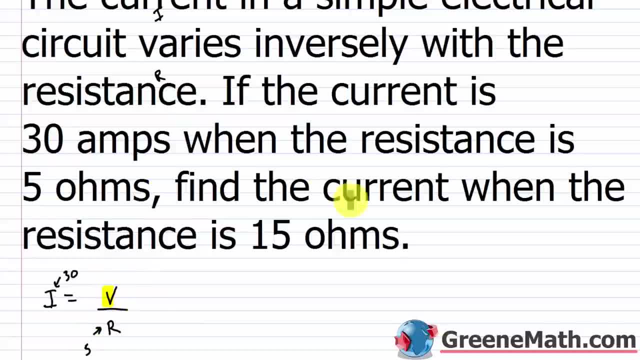 We just want to find V. We want to find V and then apply it to that second scenario that gives us. So let's solve for that. 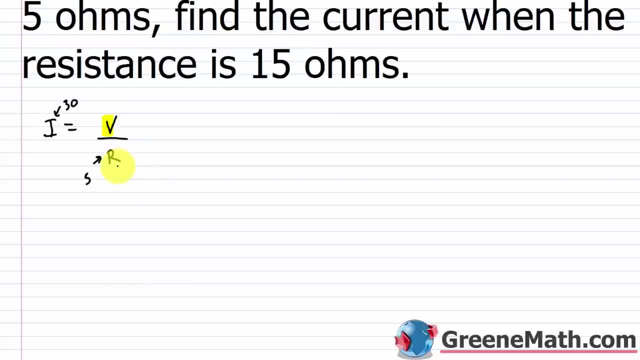 So what I would do here, I would multiply. We'd have 30 equals V over 5. 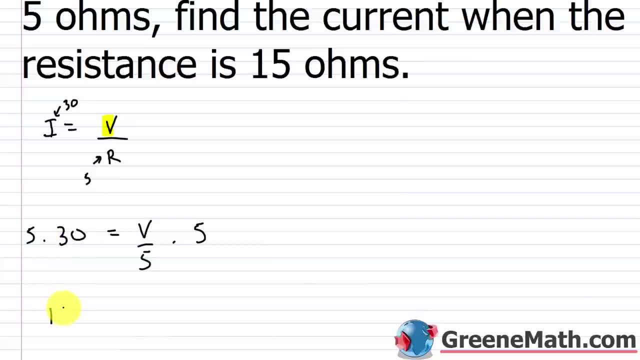 Multiply both sides of the equation by 5. And I would get 150 is equal to V. So that's my voltage. That's going to stay the same. 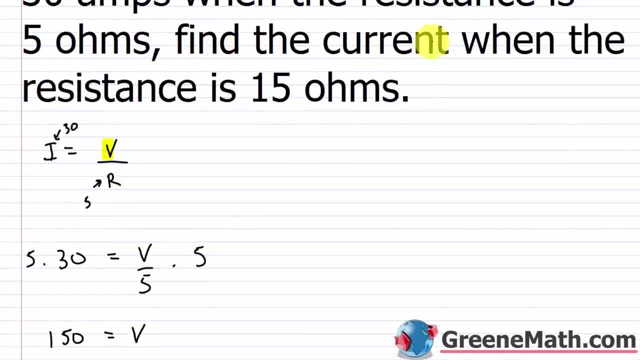 Okay. So now in the next scenario, we want to find the current when the resistance is 15 ohms. 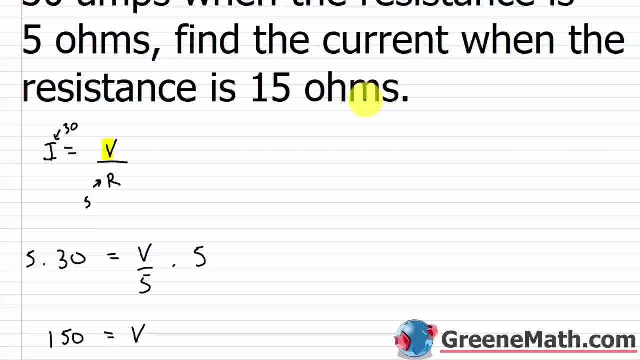 Now, the resistance goes up. That means that the current is going to go down, right? It's inverse variation. 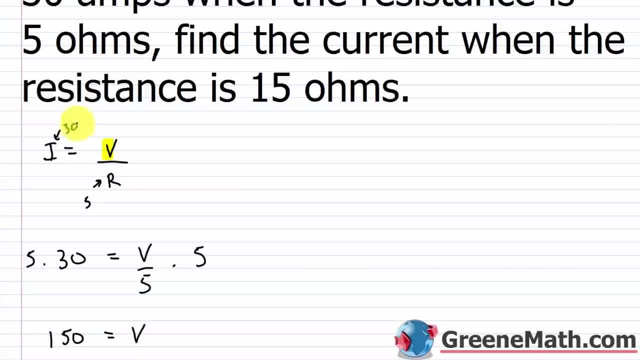 So we're looking for a smaller value than 30 here, right? So if I plug in, I have I is equal to. I know that my voltage, which is V that's on top is 150 and they're giving me this 15 for the resistance. Pretty easy to do this here. 150 divided by 15 is 10. 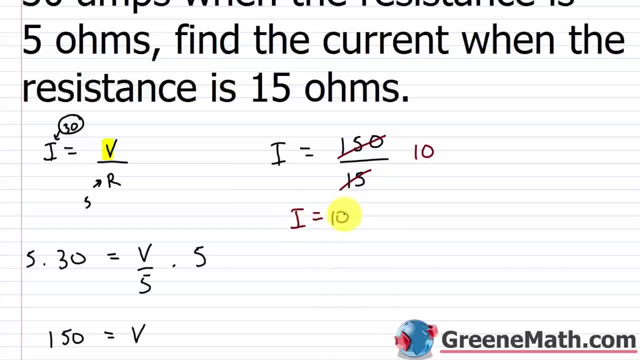 So I is equal to 10 in this scenario because it's a word problem. We probably want to put a nice little sentence there and say that the current is 10 amps. 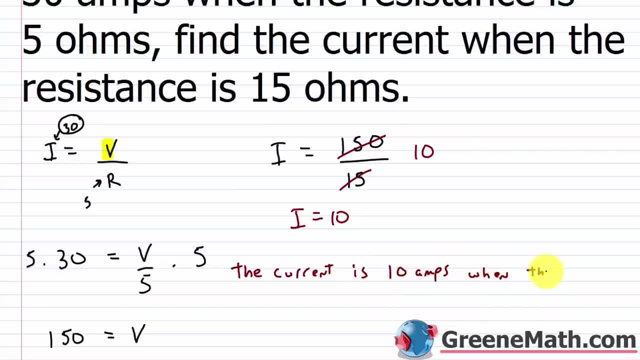 When the resistance is 15 ohms, okay. And one of the things you can notice about this again, it's inverse variation. 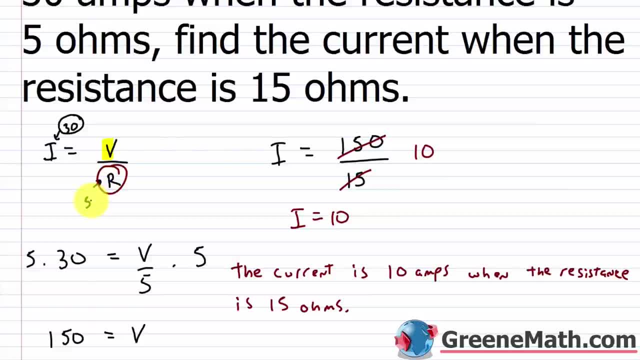 So as R increased, it went from 5 to 15, the I or the current decreased. It went from 30 to 10. So that's consistent with what we know about inverse variation. All right. 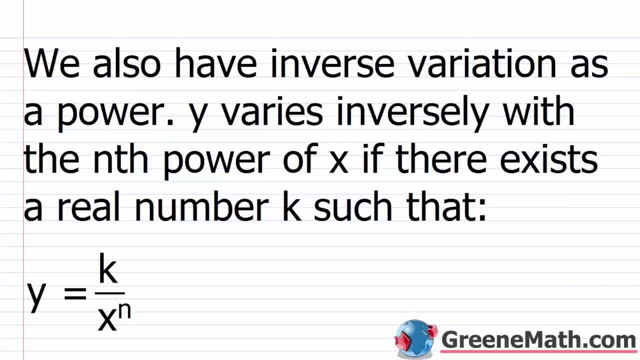 So to kind of wrap up the lesson, we're also going to see inverse variation as a power. So this is no more difficult. It's just plugging things in, figuring out what K is, and then following up with your scenario that they're giving you. 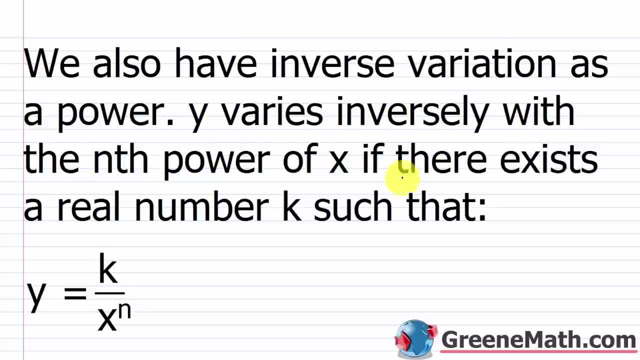 So Y varies inversely with the nth power of X if there exists a real number K such that Y equals K, the constant of variation over X to the nth power. 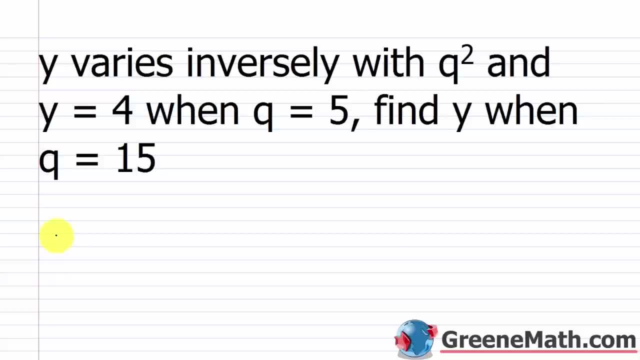 So Y varies inversely with Q squared. So Y is equal to your variable in the place of X, as you'd normally get it, is now Q. So you just put Y equals K over Q squared. 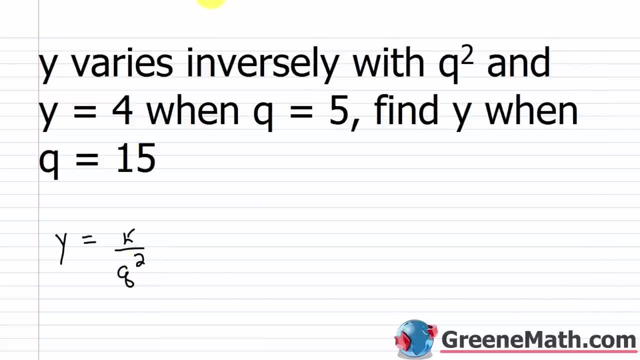 And then we're given the scenario where Y is equal to 4. So Y is going to be 4 when Q is going to be 5. So we're going to use this to solve for K, and then we can figure out what this guy is. So Y is 4 when Q is 5. 5 squared is 20. So K over 25. Obviously K there is 100, right? If I multiply both sides by 25, I'm going to get that K equals 100. 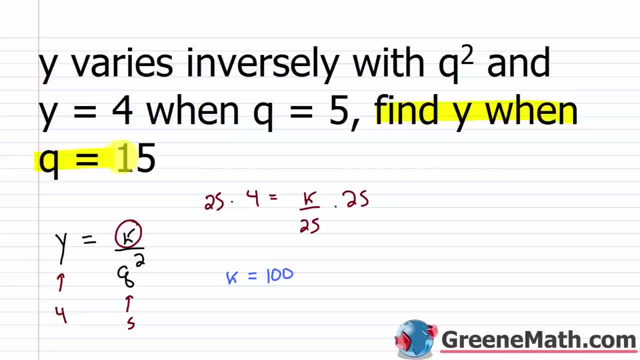 So now we want to do this scenario where we find Y when Q equals 15. So I'd be plugging in a 15 there. 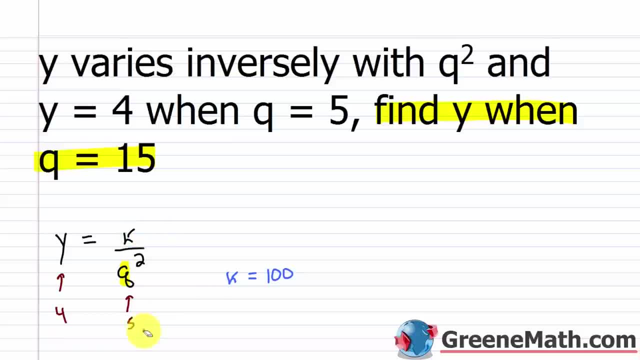 So let me erase this real quick, just get a little room going. 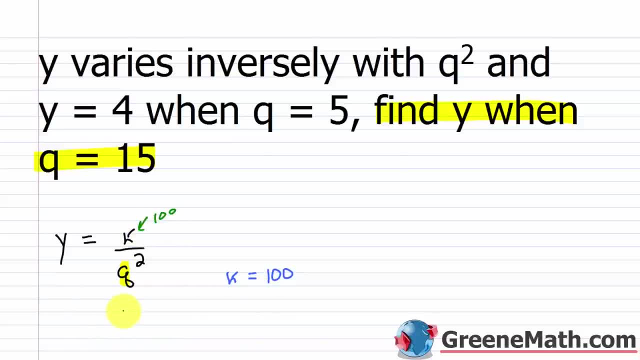 So I know K is 100. So 100 is going to get plugged in there. And Q is 15. 15 is going there. And so what I'm going to have is Y is equal to 100 over 15 squared. 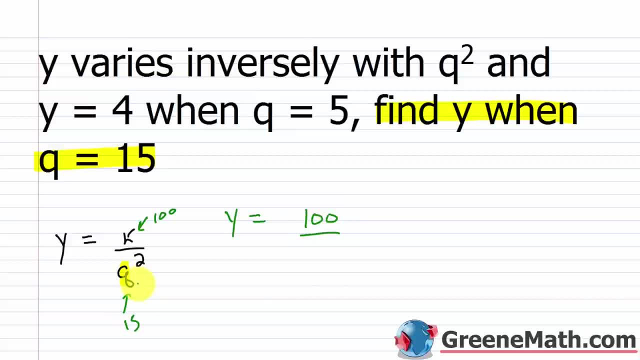 Now a lot of you don't know 15 squared is 225 yet, but by the time you finish Algebra 2, you're going to know that for sure. 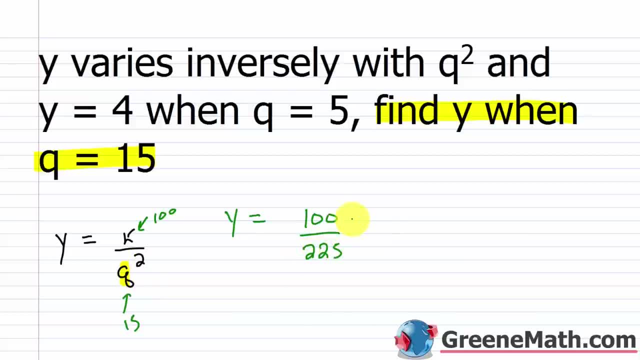 So 15 squared is 225. All right, we can reduce this fraction. So each of these is going to be divisible by 25. 100 divided by 25 is going to be 4. 225 is going to be 4. 225 is going to be 5. 225 is going to be 5. 225 divided by 25 is going to be 9. So this ends up being 4 ninths as my answer. 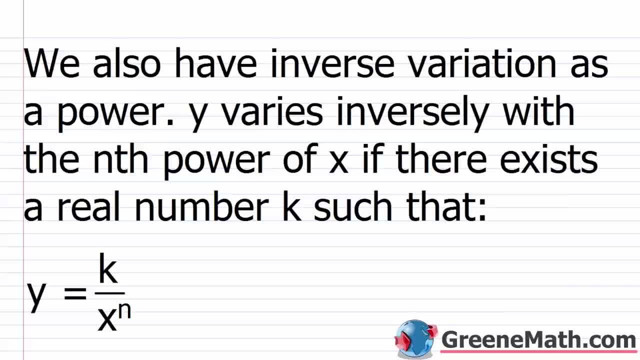 We're also going to see Inverse variation as a power, So this is no more difficult. It's just plugging things in: Figuring out what K is And then following up with your scenario That they're giving you. So Y varies inversely with the. 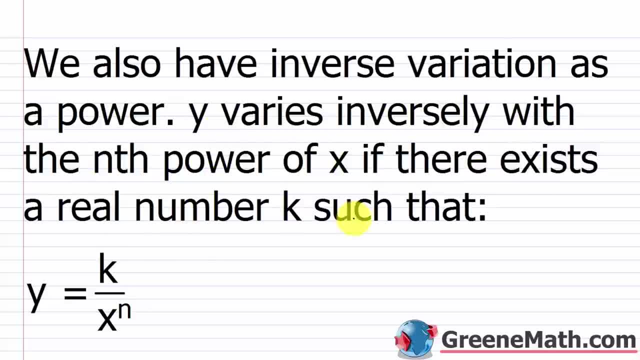 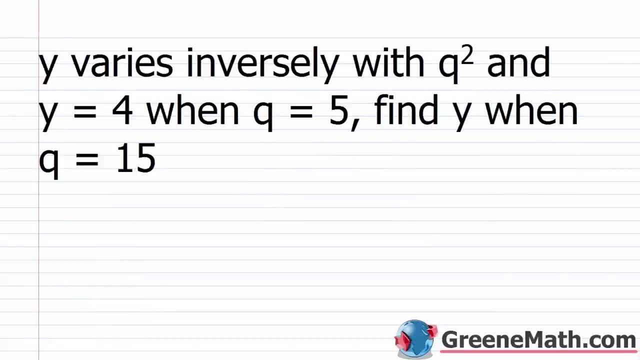 Nth power of X. If there exists a real number, K, Then we can approach that Y equals K, The constant of variation Over X to the nth power. So Y varies inversely with Q squared, So Y is equal to. 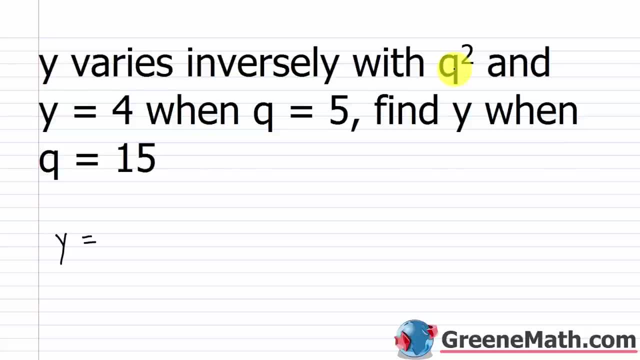 Your variable. in the place of X, as you'd normally get, it, Is now Q. So you just put Y equals K over Q squared, And then we're given the scenario where Y is equal to 4.. So Y is going to be 4.. 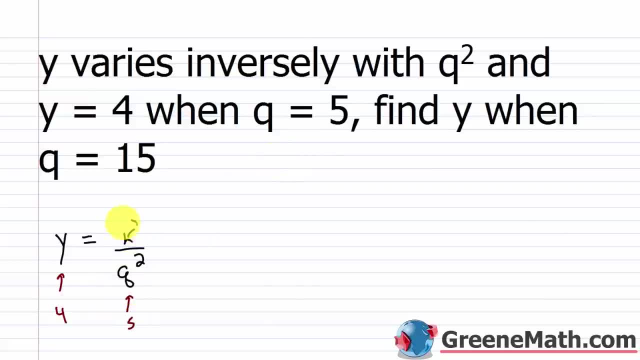 When Q is going to be 5.. So we're going to use this to solve for K And then we can figure out what this guy is. So Y is 4.. When Q is 5. 5 squared is 25.. 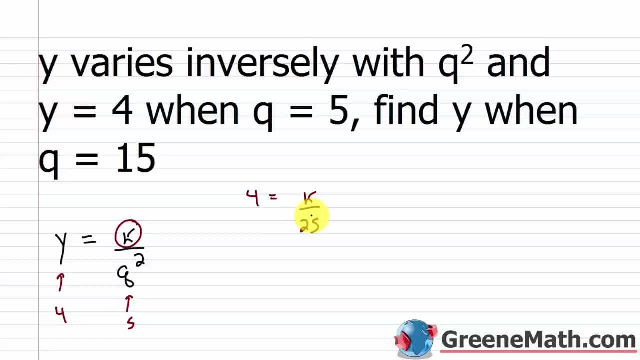 So K over 25.. Obviously K there is 100. If I multiply both sides by 25. I'm going to get that K equals 100.. So now we want to do this scenario Where we find Y When Q equals 15.. 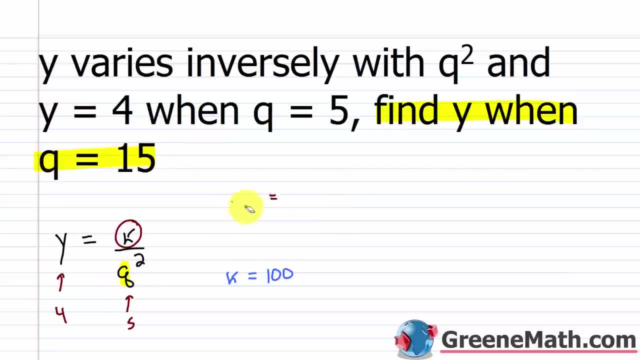 There. So let me erase this real quick. Just get a little room going. So I know K is 100. So 100 is going to get plugged in there And Q is 15.. 15 is going there, And so what I'm going to have is: 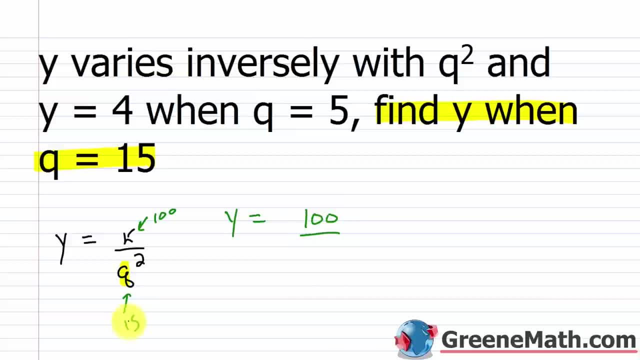 Y is equal to 100 over 15 squared. Now, a lot of you don't know 15 squared is 225 yet, But by the time you finish, algebra 2.. You're going to know that for sure: 225.. 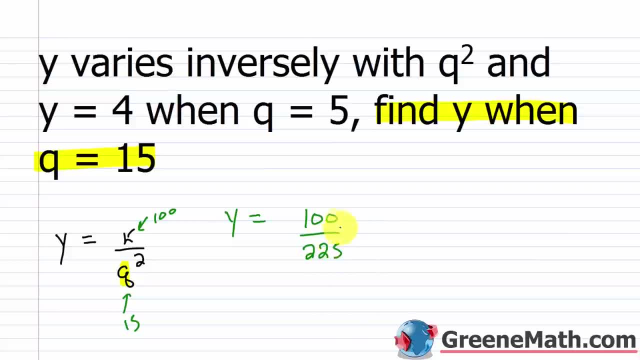 Alright, we can reduce this fraction. So each of these is going to be divisible by 25.. 100 divided by 25. Is going to be 4.. 225 divided by 25. Is going to be 9.. So this ends up being 4 9ths. 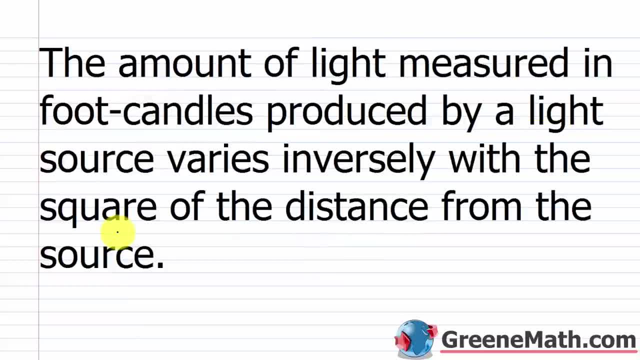 As my answer. Alright, so let's wrap up the lesson By looking at a word problem. So we have that the amount of light measured in foot candles Produced by a light source Varies inversely With the square of the distance. 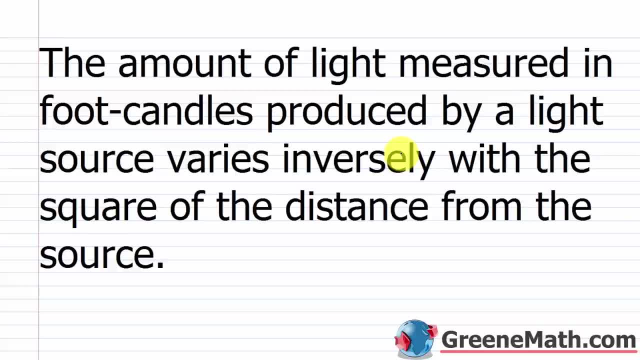 From the source. So let's just label things. I'm going to say that the amount of light measured in foot candles Produced by a light source, Let's just go ahead and say that's L, And this varies inversely With the square of the distance from the source. 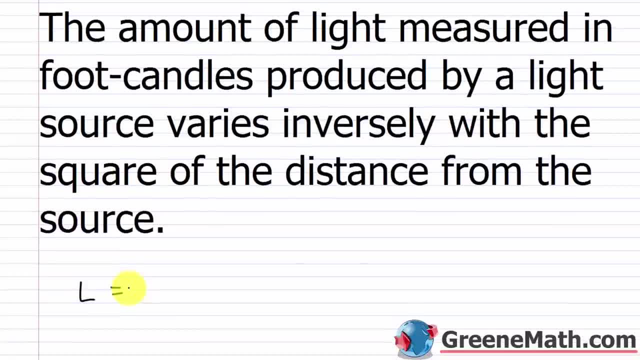 So let's say the distance from the source. Let's say that's D And that's going to be squared. So we'll put D squared down here, And then for my constant of variation I'm just going to use K. Alright, nice and simple. 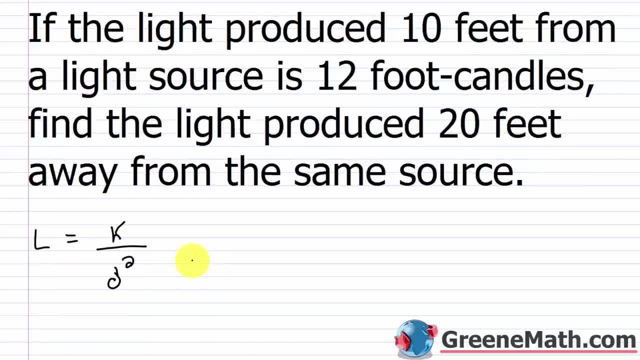 I'm going to copy this Because we're going to need it. Okay, so if the light produced 10 feet from a light source, So that's the distance, So I'm going to plug in a 10 for D. there Is 12 foot candles. 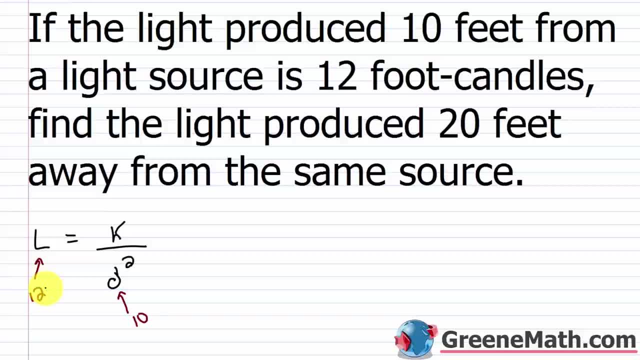 So this is going to be 12. Find the light produced 20 feet away From the same source. So what we want to do Again is just plug in this Find K And then figure out what this second scenario is That they're giving us. 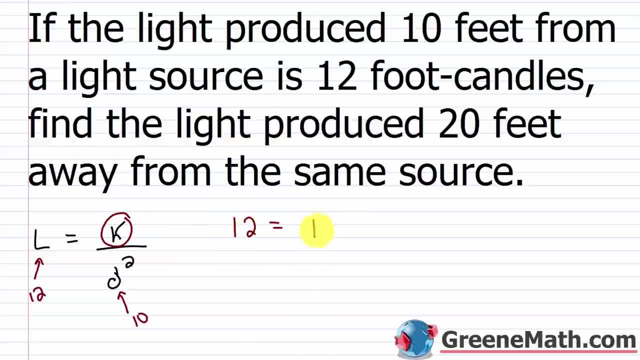 And then a 12 for L, I'd have. 12 is equal to, You'd have K over 10 squared, Which is 100.. To isolate K, I'd multiply both sides by 100. And so this would cancel with this. 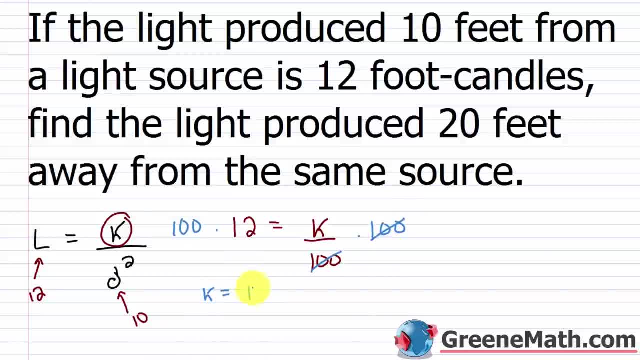 And you would get: K is equal to 1200.. Now Let me erase all this real quick. And in this second scenario, The one that we need to figure out Is find the light produced 20 feet away from the same source. 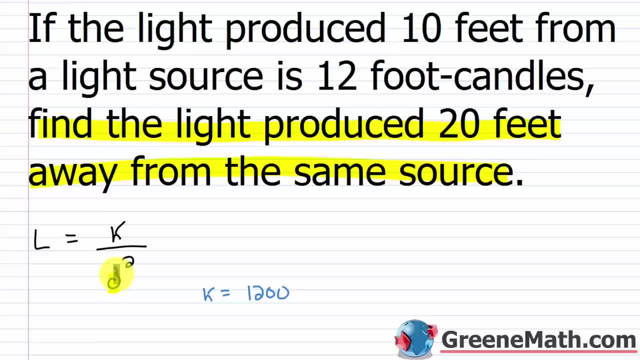 So now the distance, The D part, Is going to be a 20.. So plug in a 20 there. And I know that K is still 1200. So this is 1200.. So the L Is going to be equal to. 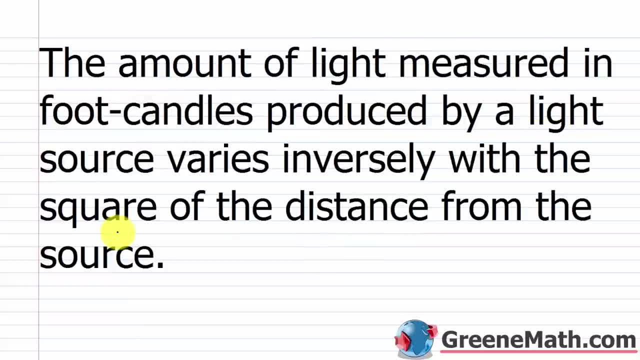 All right, so let's wrap up the lesson by looking at a word problem. So we have that the amount of light measured in foot candles produced by a light source 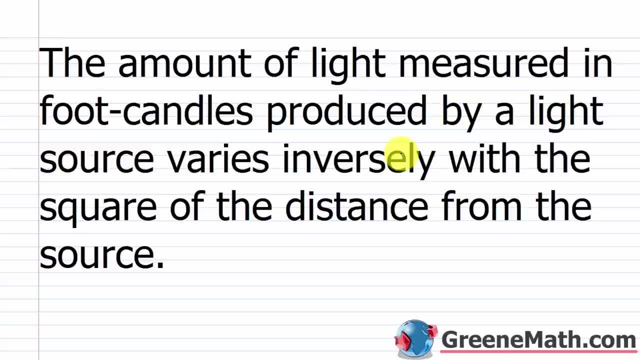 varies inversely with the square of the distance from the source. 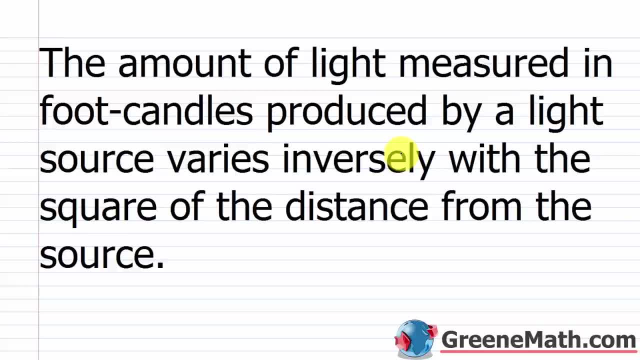 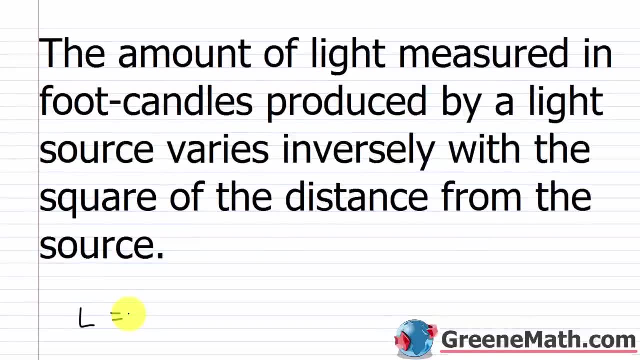 So let's just label things. I'm going to say that the amount of light measured in foot candles produced by a light source, let's just go ahead and just say that's L. And this varies inversely with the square of the distance from the source. So let's say the distance from the source, let's say that's D, and that's going to be squared. 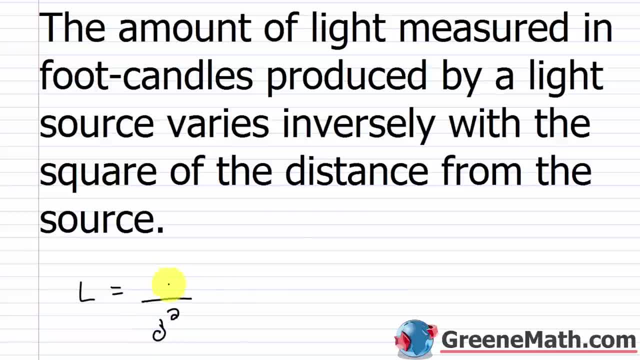 So we'll put D squared down here. And then for my constant of variation, I'm just going to use K. All right, nice and simple. All right, so let's copy this because we're going to need it. 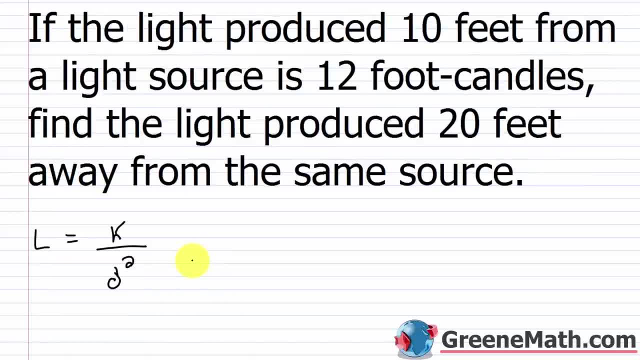 Okay, so if the light produced 10 feet from a light source, so that's the distance. So I'm going to plug in a 10 for D there. All right. So 12 foot candles, so this is going to be 12. 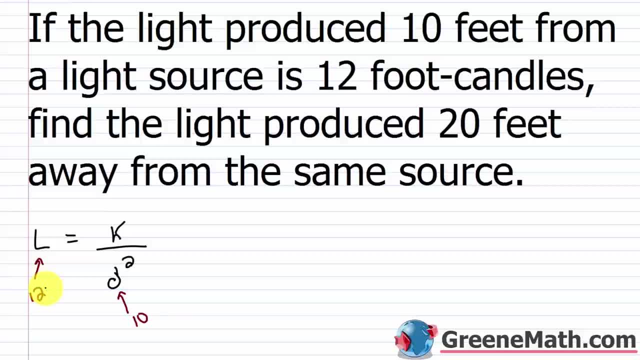 Find the light produced 20 feet away from the same source. So what we want to do, again, is just plug in this, find K, and then figure out what this second scenario is that they're giving us. 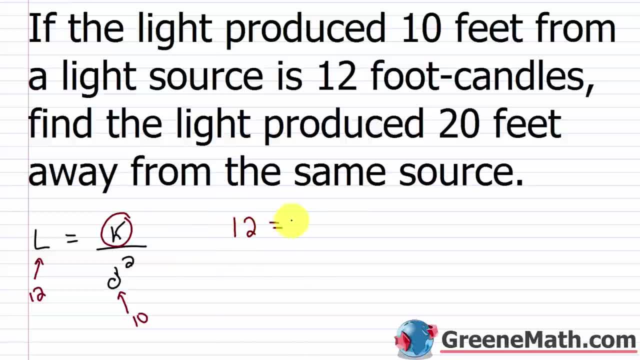 So if I plugged in a 12 for L, I'd have 12 is equal to, you'd have K over 10 squared, which is 100. To isolate K, I'd multiply both sides by 100. All right. 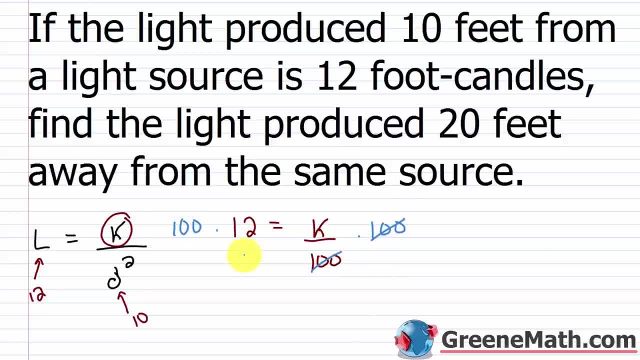 And so this would cancel with this, and you would get K is equal to 1,200. 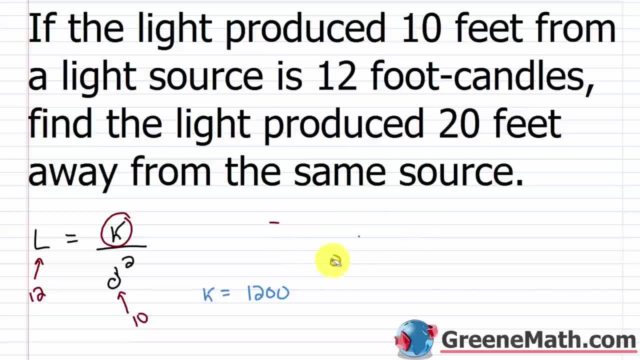 Now, let me erase all this real quick. 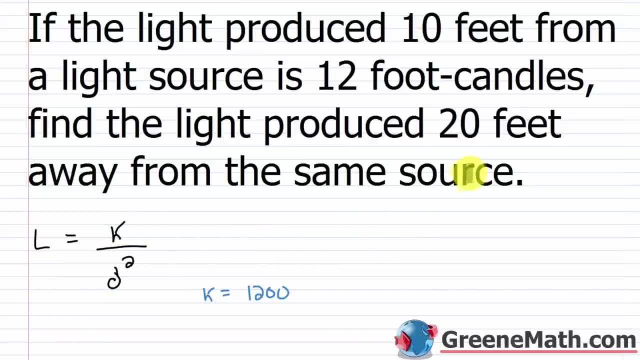 And in this second scenario, the one that we need to figure out, it says find the light produced 20 feet away from the same source. So now the distance, the D part, is going to be a 20. 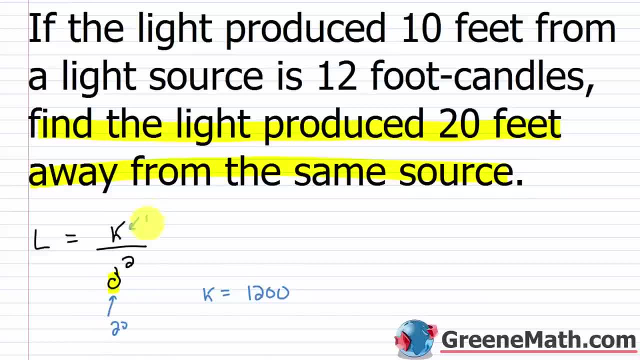 So I plug in a 20 there. And I know that K is still 1,200. So this is 1,200. So the L is going to be equal to 1,200 over 20 squared. Now, 20 squared is 400. So 400. And I know that I can cancel two zeros with two zeros. It's like canceling out a common factor of 100. And then 12 divided by 4 is 3. 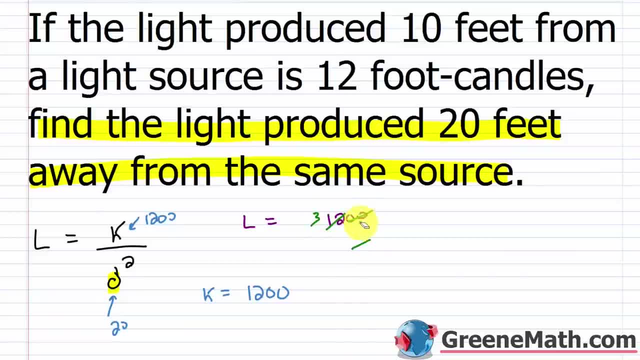 So the L here, or the light produced, is going to be 3. And in terms of units, it would be 3 foot candles. So let's go ahead and write that down. All right. 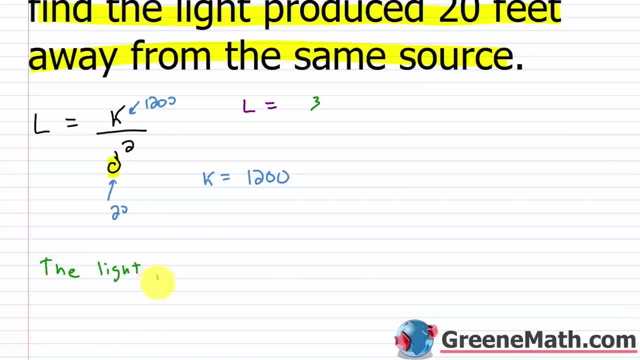 Let's go ahead and write that the light produced 20 feet away from the light source is 3 foot candles. 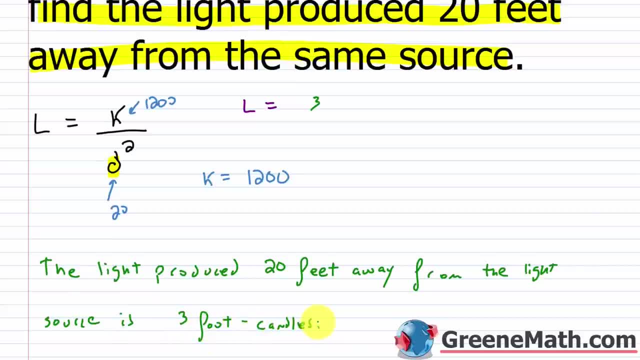 Hello, and welcome to Algebra 1, Lesson 52. 1. 2. 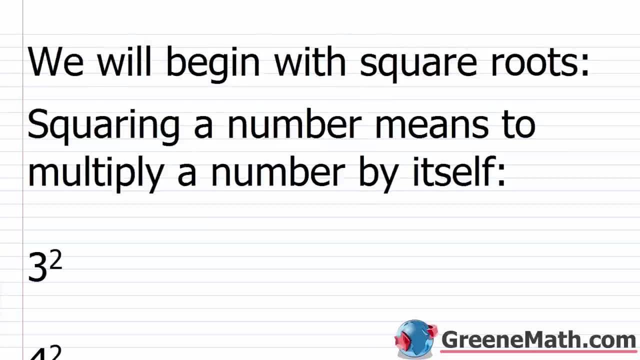 3. 4. 5. 6. 7. 8. 9. 10. 11. 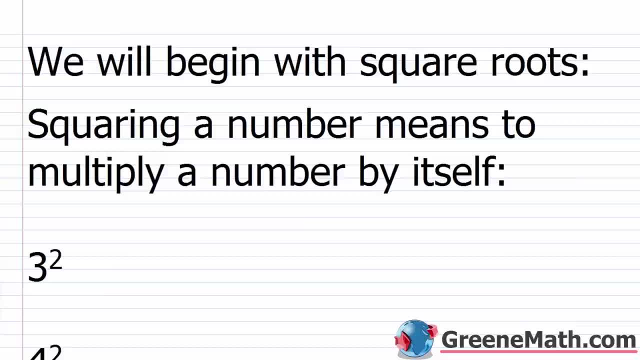 12. 12. 13. 14. 15. 16. 17. 18. 19. 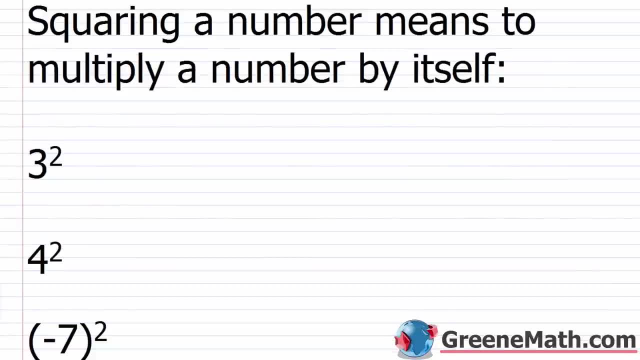 20. 21. 22. 22. 23. 24. 25. 26. 27. 28. 29. 30. 31. 32. 33. 34. 35. 36. 37. 38. 39. 40. 41. 42. 42. 43. 44. 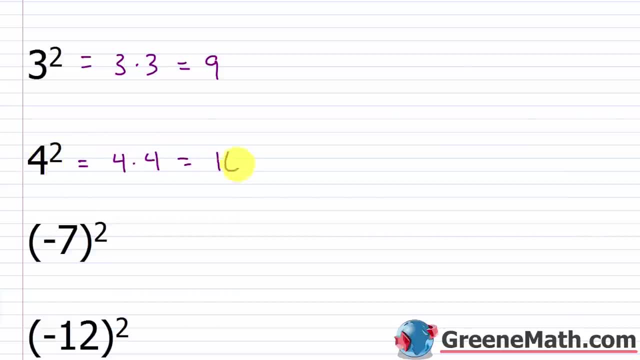 44. 45. 46. 47. 48. 49. 50. 51. 52. 52. 53. 52. 53. 54. 55. 56. 57. 58. 59. 60. 61. 62. 62. 63. 63. 64. 65. 67. 68. 67. 68. 69. 69. 70. 71. 72. 72. 73. 73. 74. 74. 75. 75. 76. 77. 78. 78. 79. 79. 80. 80. 81. 81. 82. 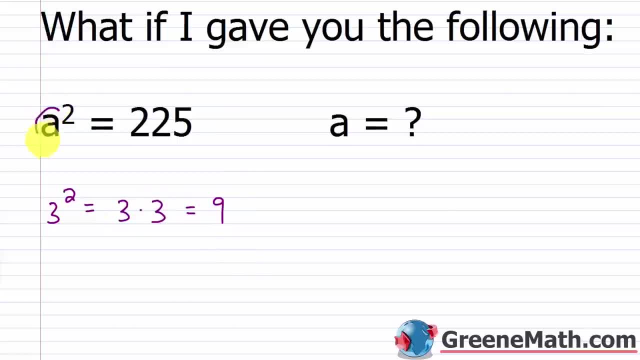 82. 83. 83. 84. 84. 85. 86. 87. 86. 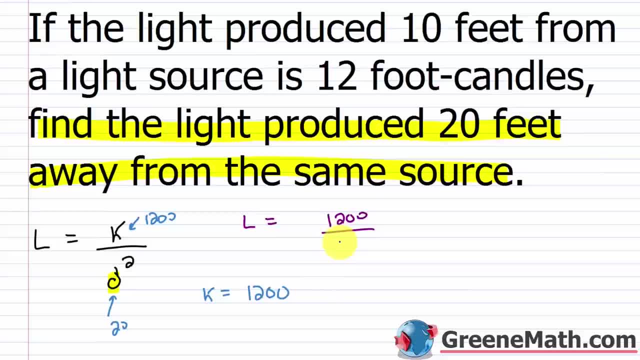 1200 over 20 squared. Now 20 squared is 400.. So 400. And I know that I can cancel Two zeros with two zeros. It's like canceling out a common factor of 100. And then 12 divided by 4.. 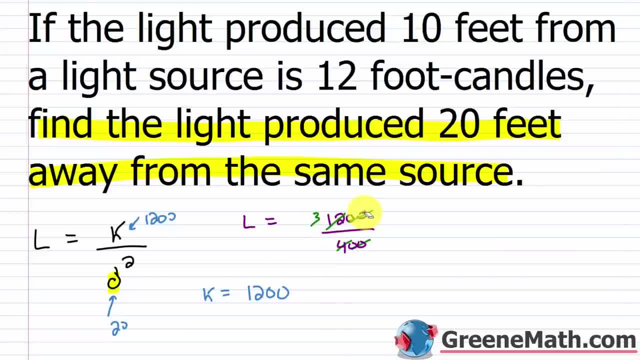 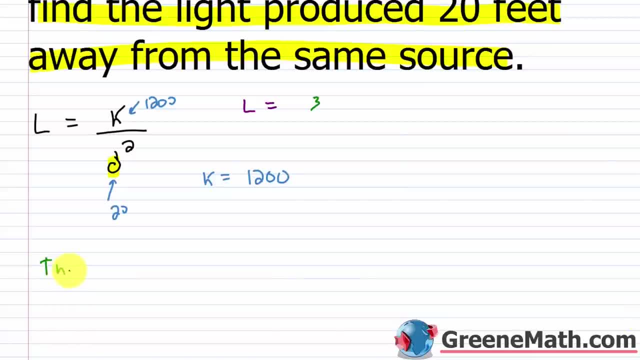 Is 3.. So the L here, or the light produced, Is going to be 3. And in terms of units it would be 3 foot candles. So let's go ahead and write that The light Produced 20 feet away. 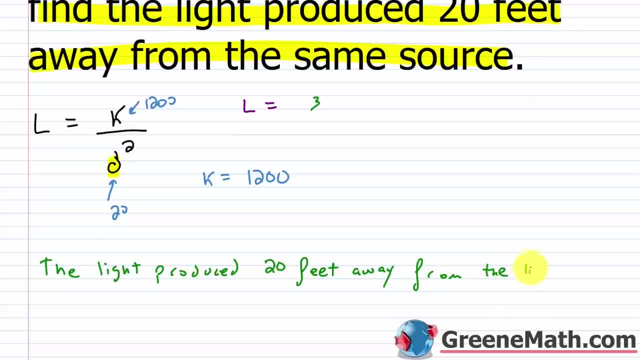 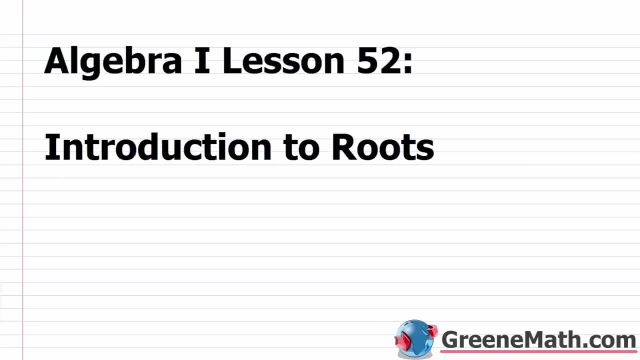 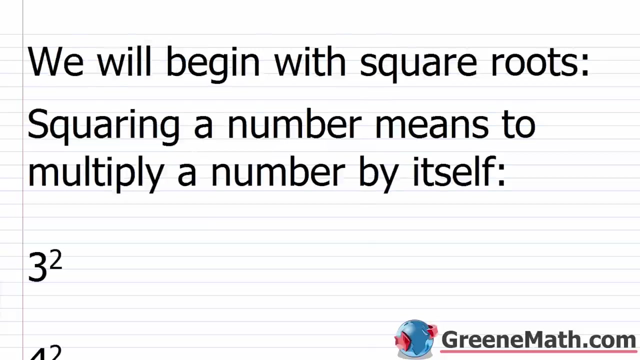 From the light source Is 3 foot candles. Hello and welcome to Algebra 1, lesson 52.. In this video we're going to have an Introduction to roots, So I know for some of you You've learned about square roots. 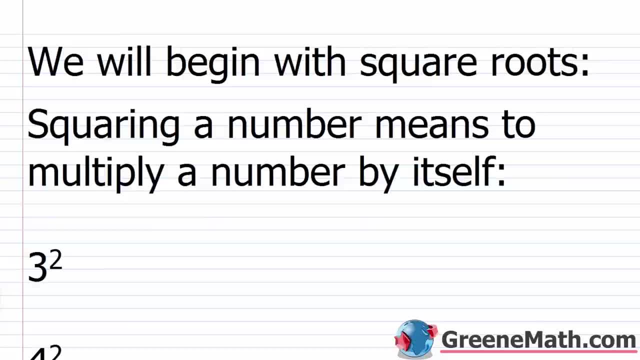 In a previous course, But for others, you've had no exposure to it What so ever. So we're going to just begin by talking about square roots. I'm going to pretend like you have No prior knowledge of it And we're going to start from scratch. 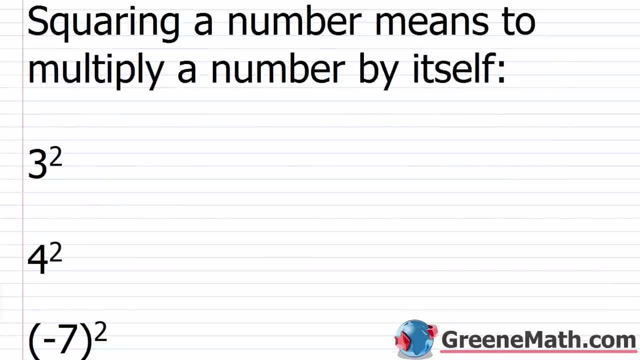 Alright. so I want you to think back To when we first started talking about exponents And we learned what it meant to square a number. So squaring a number Means to multiply a number By itself. Basically, it's when you have an exponent of 2.. 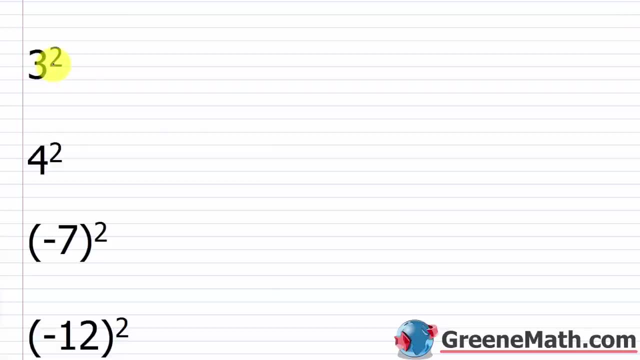 So for these four examples here, We have 3 squared, So we know at this point that this is what It's: 3 times 3. Or 9.. If I have 4 squared, 4 times 4. Or 16.. 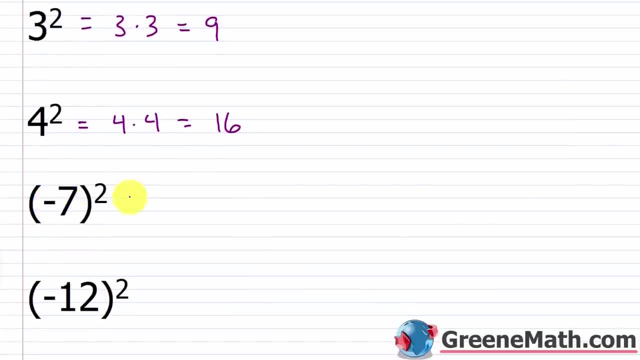 If I have negative 7 squared With the negative and the 7 inside of parenthesis, This is negative 7.. Times negative 7.. Which is positive: 49.. And then, if I have negative 12 squared Again with the negative and the 12 inside of parenthesis, 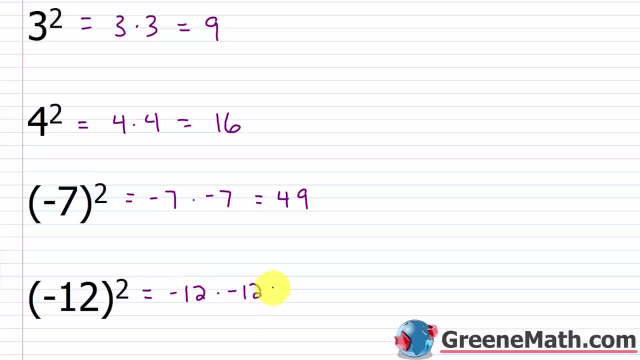 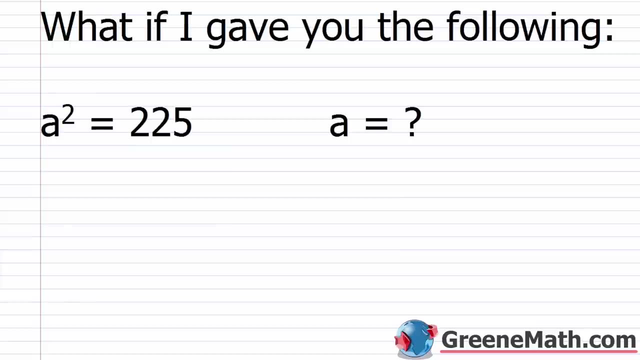 This is negative 12.. Times, negative 12.. Which is positive: 144.. Now what if I gave you The following scenario? I have here that a squared, So something squared, Is equal to 225.. What is the value for a? 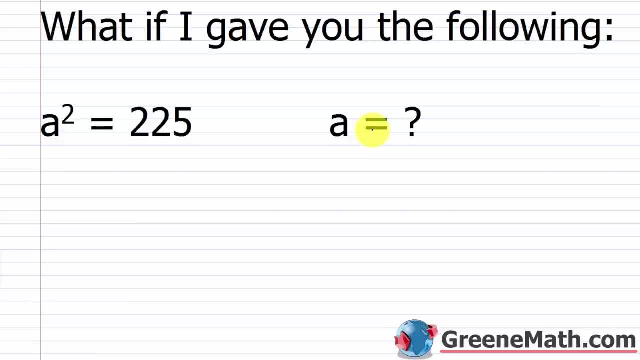 So you might be thinking: How would I go about doing that? Well, let's just go back to a simple example. We saw that 3 squared Was equal to 9.. Why is it equal to 9?? Well, I can further break this down. 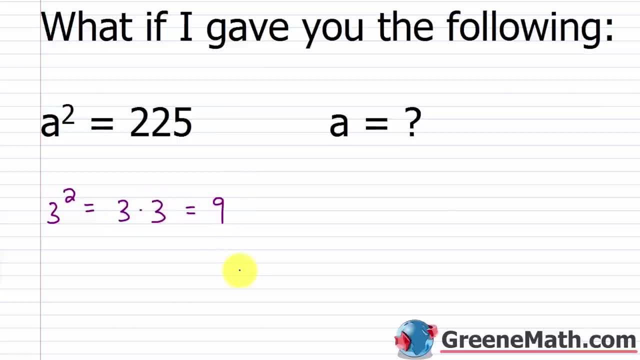 And say it's 3 times 3.. Which equals 9.. Now, if I think about a number, A number When multiplied by itself- So in other words this would translate to A squared- is equal to a Times a, Which equals 225.. 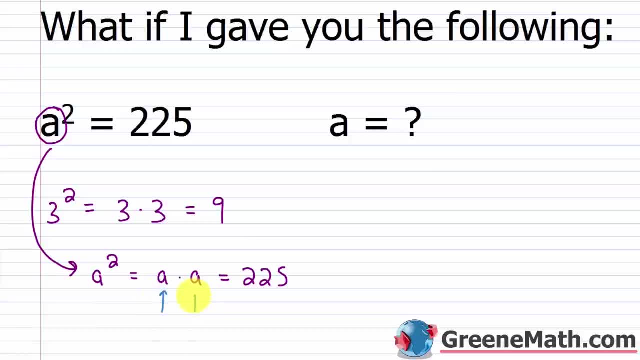 So I've got to think about a number That, when multiplied by itself, Is going to give me 225.. Can you think of a number? Well, if you can't, You can just break 225 down Using a factor tree, So it ends in 5.. 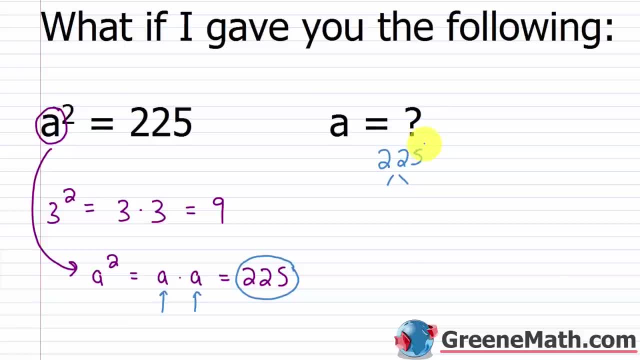 So that means it's divisible by 5.. 225 divided by 5. Is 45. So let's write 45. Times 5. And then 5 is going to be prime. So let's circle that, And then 45 can be further broken down. 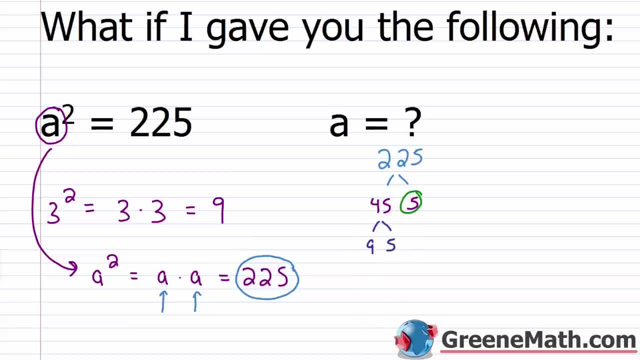 Into 9 times 5.. 5 is prime, So let's circle that. And then 9 is 3 times 3.. So 3 times 3.. And those are each prime, So let's circle those. And what can I see here? 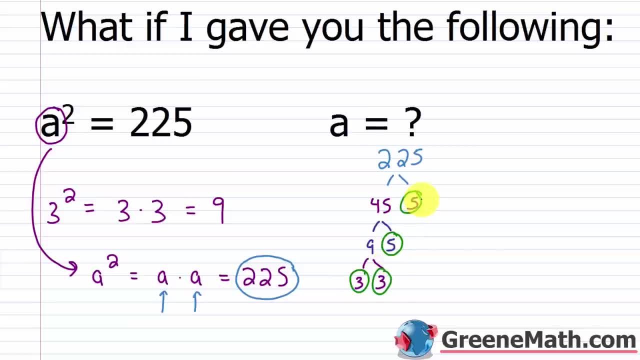 I have 3 times 5 or 15.. So 225. Is 15 times 15.. So we've found a number That, when multiplied by itself, Is going to give us 225.. So where we have a question mark here: 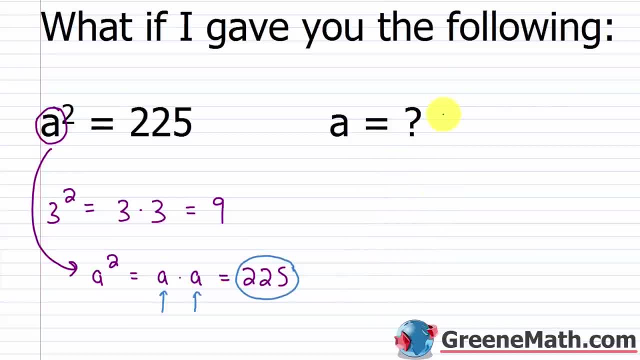 Let me erase all this. I can put a value of 15.. Now some of you will be screaming At this point. going: Well, what about negative 15?? If I took negative 15. And I multiplied it by negative 15.. 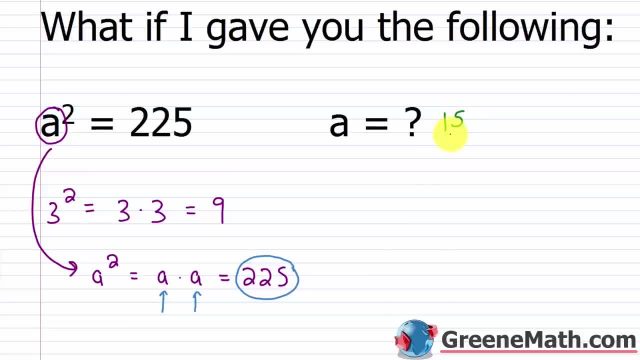 I would also get 225.. So you'd be correct there. It could be 15, or It could also be negative 15.. If I had negative 15. And that was squared, This would be negative 15.. Times negative 15.. 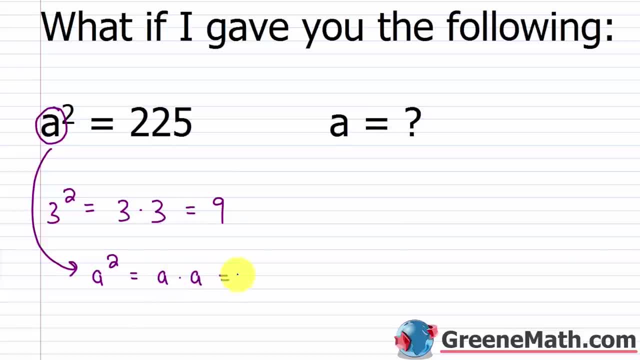 87. 88. 88. 89. 90. 91. 92. 92. 93. 92. 08. 07. 1. 08. 07. 08. 08. 07. 0 த. 0ITE. 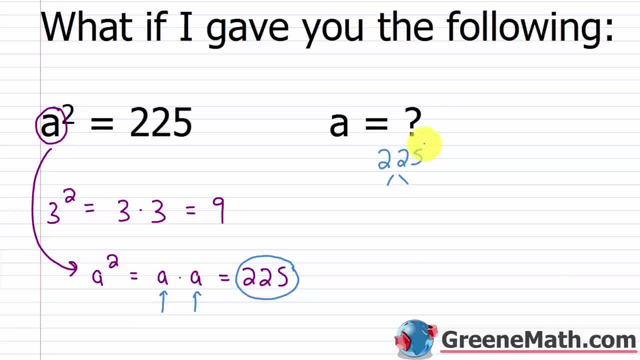 0 morgen . 08. 09. 09. 09. 10. 010. 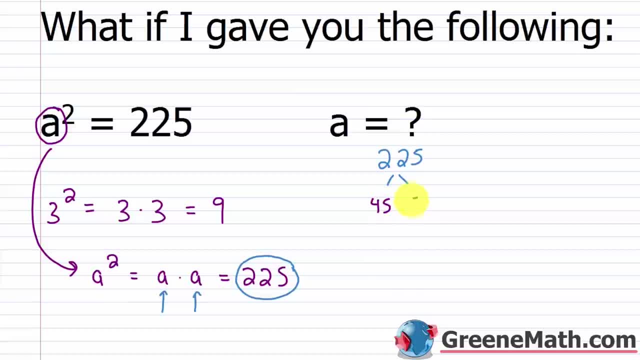 10. 100. 00. 00. 017. 10Stud. 14. Itопrof. Mr. 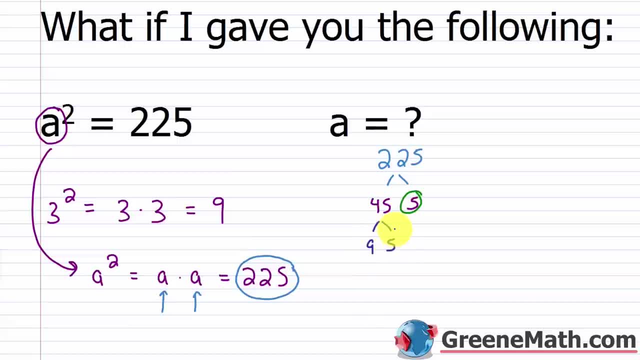 crown. further broken down into 9 times 5. 5 is prime, so let's circle that. And then 9 is 3 times 3. So 3 times 3. And those are each prime, so let's circle those. And what can I see here? I have 3 times 5 or 15, and then I have 3 times 5 again or 15. So 225 is 15 times 15. So we've found a number that when multiplied by itself is going to give us 225. So where we have a question mark here, let me erase all this, I can put a value of 15. Now some of you will be screaming at this point going, well what about negative 15? If I took negative 15 and I multiplied it by negative 15, I would also get 225. So you'd be correct there. So a could be 15 or it could also be negative 15, right? If I had negative 15, I would also get 225. So you'd be correct there. 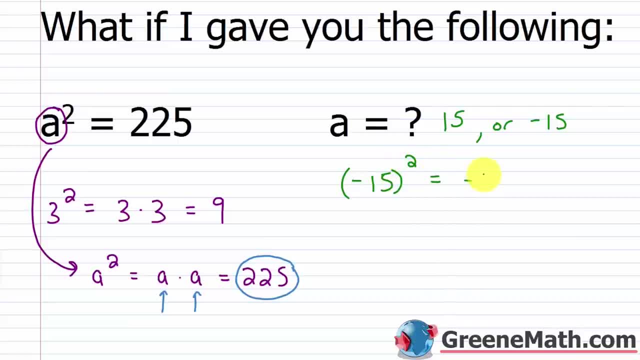 So if I took negative 15 and that was squared, this would be negative 15 times negative 15, which would also give me a positive 225. So when we think about square roots, okay, we're going to think about a positive version and a negative version, and I'm going to show you the notation for that in a minute. All right, let's take a look at another one. So we have b squared equals 100. 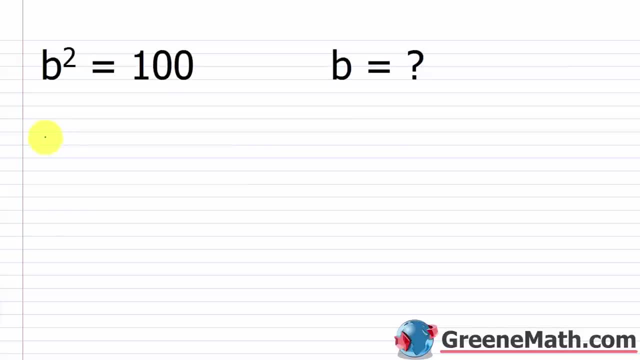 So we want to know what is the value for b. So if I took b squared and I said it's equal to, what? Let's break this down into b times b. Let's say that's equal to 100. So all I'm looking for here 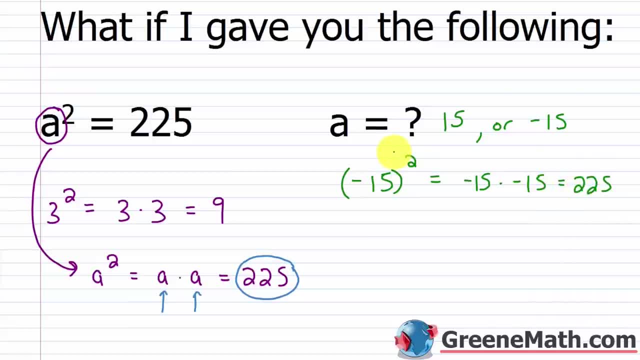 Which would also give me a positive 225.. So when we think about Square roots, We're going to think about a positive version And a negative version, And I'm going to show you the notation for that in a minute. Let's take a look at another one. 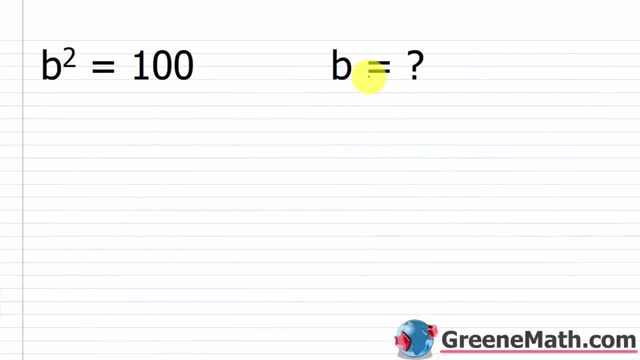 So we have: b squared equals 100. So we want to know The value for b. So if I took b squared And I said it's equal to, Let's break this down into b times b, Let's say that's equal to 100.. 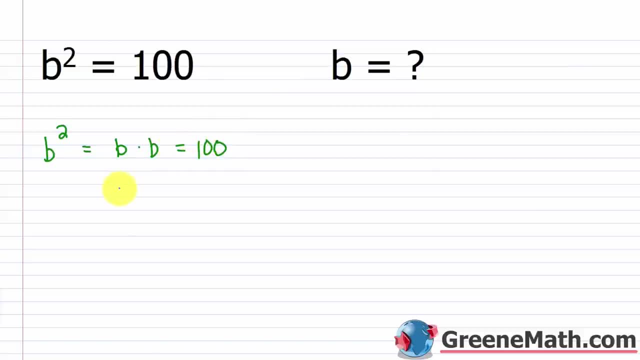 So all I'm looking for here Is: I'm looking for a number That, when multiplied by itself, Gives me 100. So again, that's easy: Just make a factor tree for 100. And most of us know that 100 is what. 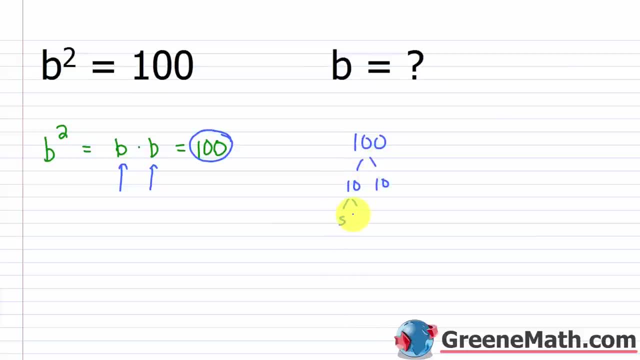 It's 10 times 10.. I don't need to go through And go all the way to 5 times 2. Because I know that 10 times 10. Is what I'm looking for. So b here would be 10.. 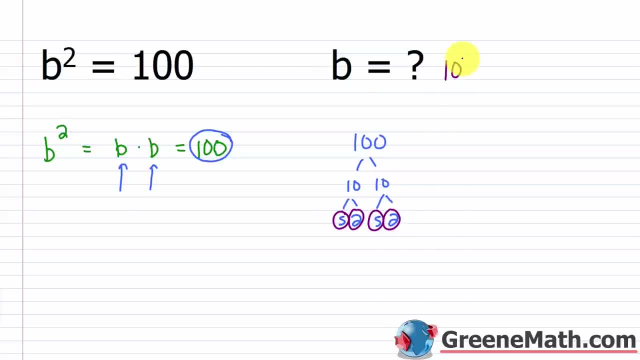 But again It could also be negative 10.. Negative 10 times negative 10. Would also give me a positive 100.. So let's think a little bit about The notation involved With what is known as a square root. So in the previous two examples, 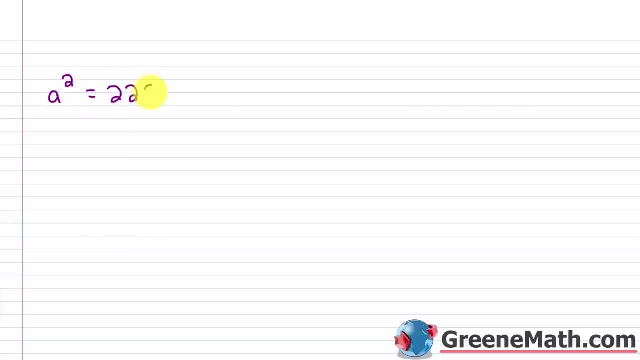 We looked at: A is equal to 225. And then we said: okay, A is equal to 15.. Or negative 15., Because 15 squared Would give me 225. And then also negative 15 squared Would give me 225 as well. 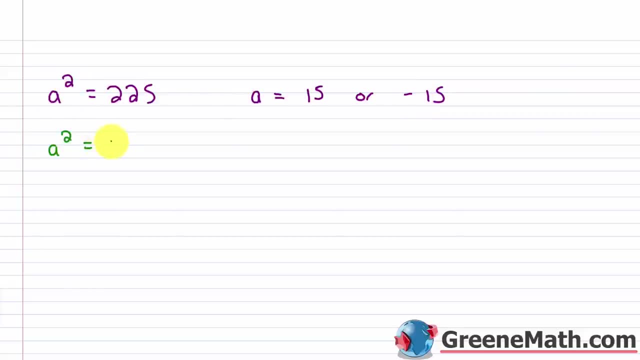 And then we looked at, A squared is equal to 100. And we said, in that case, A was equal to 10. Or it could be negative 10.. Okay, So we want to think about How this is asked to us. 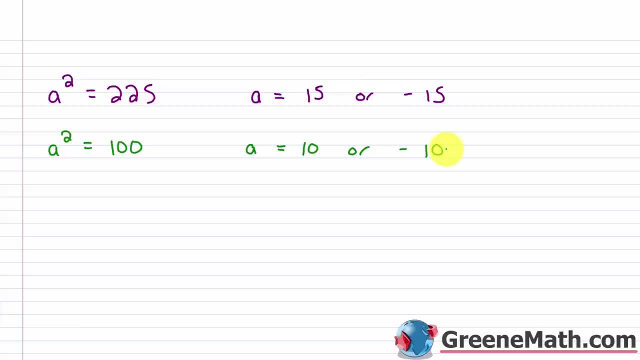 In terms of our homework Or a test. just moving forward, If I want What's known as the square root of a number, I'm going to see this symbol right here, So it looks kind of like this. So if I wanted to know, 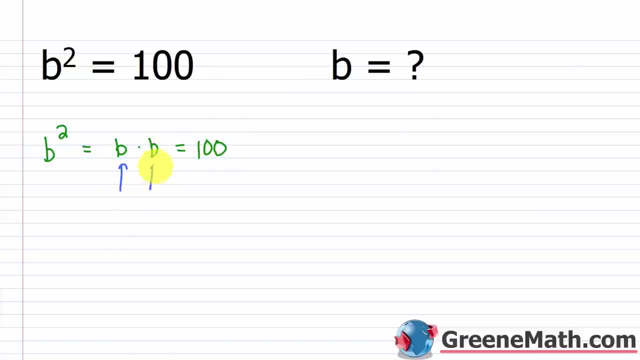 is I'm looking for a number that when multiplied by itself gives me 100. So again, that's easy. Just make a factor tree for 100. And most of us know that 100 is what? It's 10 times 10, right? I don't need to go through and go all the way to 5 times 2 and then 5 times 2 because I know that 10 times 10 is what I'm looking for, right? 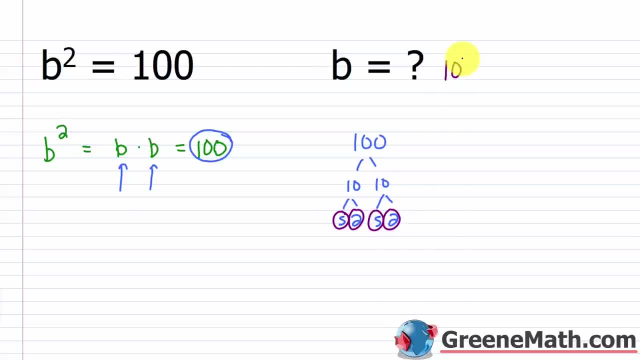 So b here would be 10. But again, it could also be negative 10, right? Negative 10 times negative 10 would also give me a positive 100. All right, so let's think a little bit about the notation involved with what is known as a square root. So in the previous two examples, we looked at, 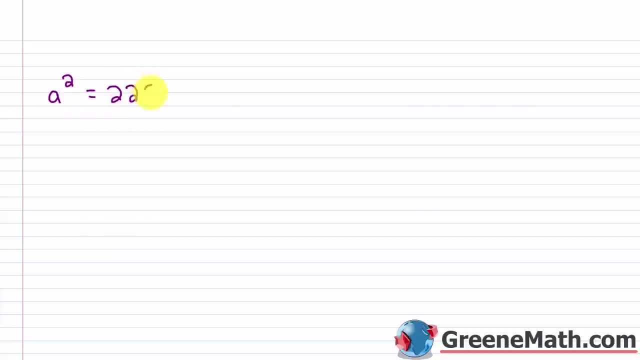 we said a squared is equal to 225. And then we said, okay, a is equal to 15 or 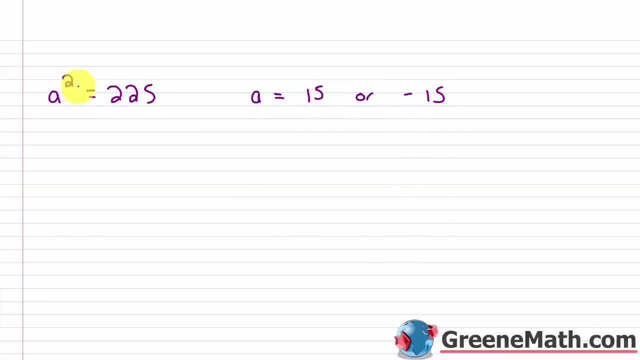 negative 10. So let's think a squared is equal to 15 or negative 10. And then we said, okay, negative 15, right? Because 15 squared would give me 225. And then also negative 15 squared would give me 225 as well. And then we looked at a squared is equal to 100. And we said in that case, a was equal to 10, or it could be negative 10. Okay. So we want to think about kind of how 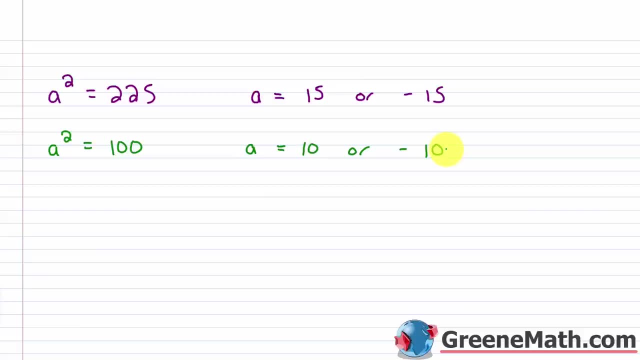 this is asked to us in terms of our homework or a test, just moving forward. If I want what's known as the square root of a number, I'm going to see this symbol right here. So it looks kind of like this. So if I wanted to know what number squared would give me 225, I would put 225 underneath this symbol. And I would say, this is the square root of 225 or what number when multiplied by itself gives me 225. We know at this point that the answer is 15. 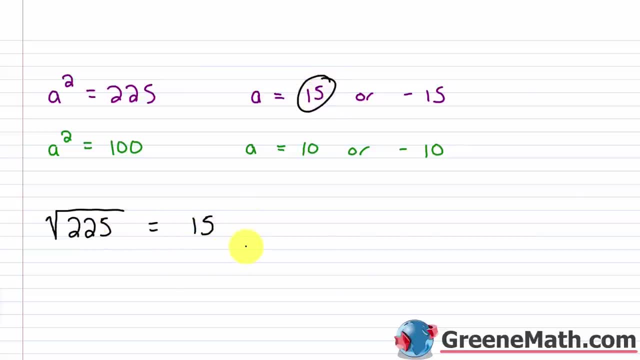 Okay. We found that here. Now, there's also a different way to kind of notate when I want negative 15. This right here 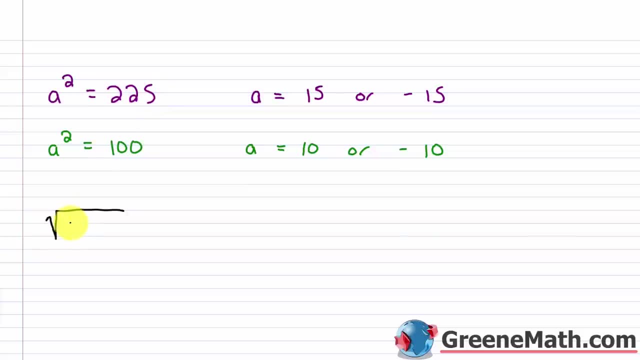 What number, squared, would give me 225. I would put 225.. Underneath this symbol And I would say: This is the square root of 225.. Or what number, When multiplied by itself, Gives me 225.. We know at this point. 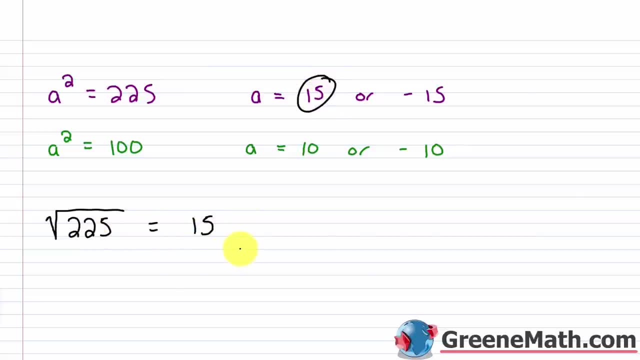 That the answer is 15.. Okay, we found that here. Now there's also a different way To kind of notate When I want negative 15. This right here is known as the principle square root Or the positive square root. 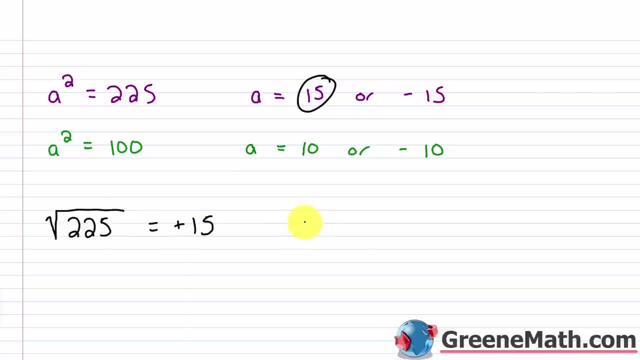 So it produces a positive here, And then we have what's known as The negative square root. So if I want this one, I put a negative out in front. So I put a negative And it's asking me for The negative of this 15.. 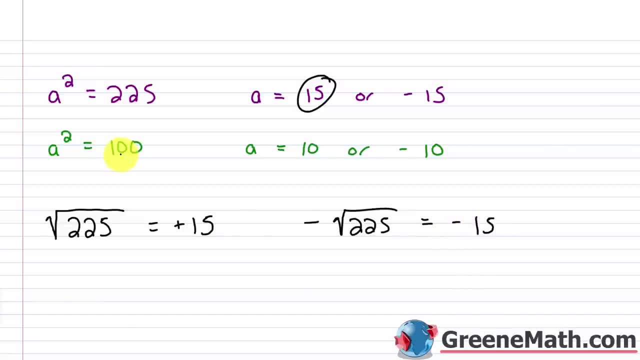 Which would be negative 15. Same thing would go for this example here. So if I want the square root of 100. This is the positive Or principle square root of 100. So that's positive, 10. And then the negative. 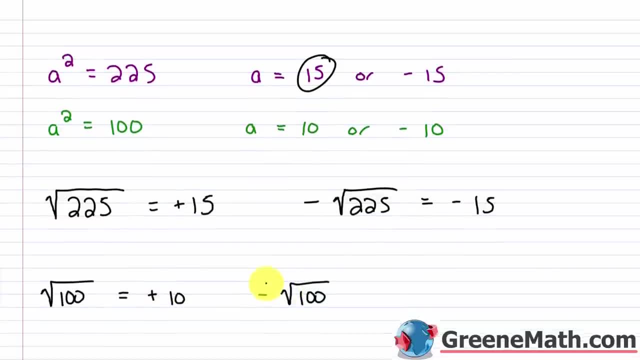 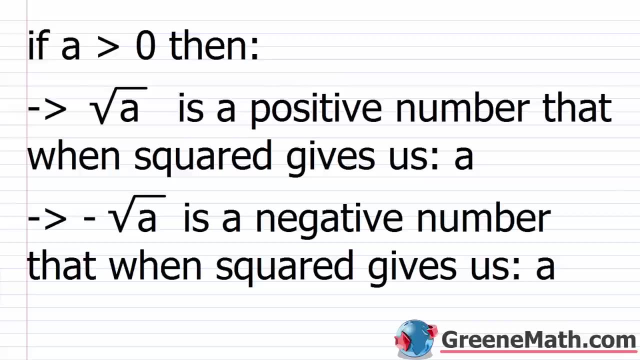 Square root of 100.. Put a negative sign out in front Would be negative 10.. So those are two different ways To kind of notate that. So that's kind of a general statement for this. If a is greater than 0.. 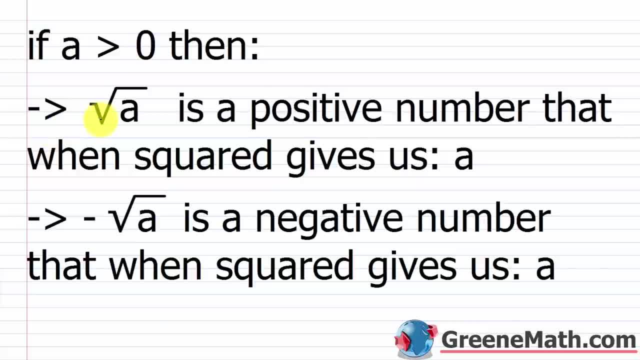 So we know that's a positive value. Then we can say that The square root of a Is a positive number, That when squared, gives us a. So in other words, If I have the square root of Again, I go back to 225.. 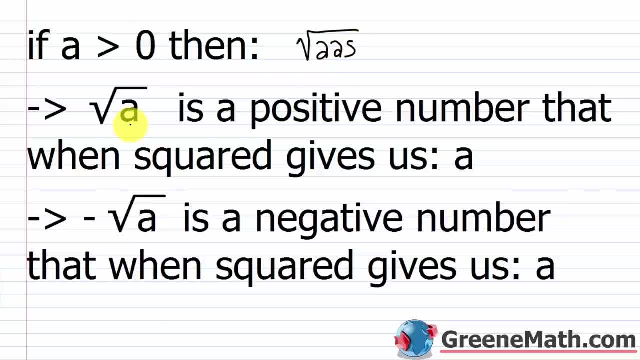 So this represents a here, So this is a positive number That, when squared, When multiplied by itself, Gives us this number back, Because 15 times 15. Would give me 225.. Or that number That's inside of that symbol back. 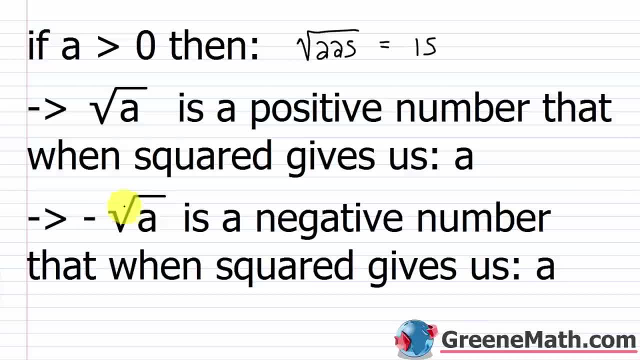 Now we have that negative Outside in front of the symbol here. Negative square root of a Is a negative number That, when squared, Gives us a. So this is a, The number inside of here. So if I did, negative square root of 225.. 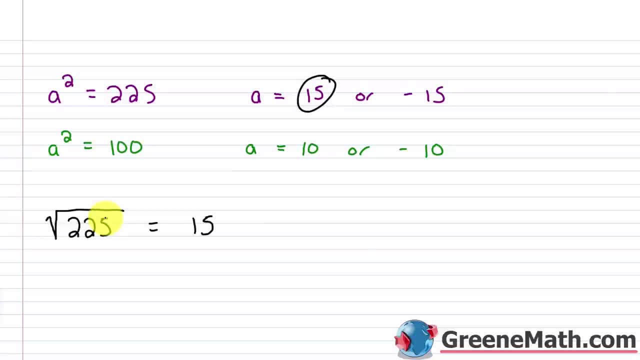 is known as the principal square root or the positive square root. So it produces a positive here. And then we have what's known as the negative square root. So if I want this one, I put a negative out in front. So I put a negative and then everything else is the same. It's just asking me for the negative of this 15, which would be negative 15. Okay. Same thing would go for the negative of this 15. So I put a negative and then everything else is the same. 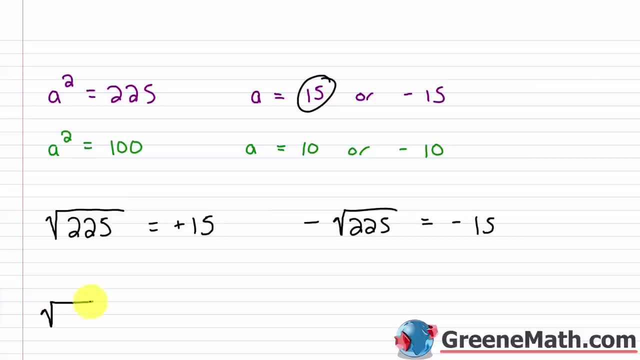 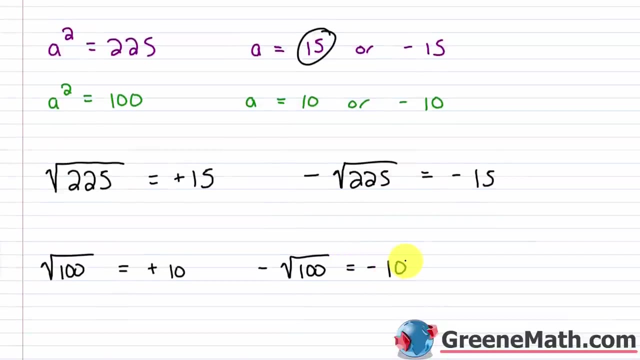 So if I want the square root of 100, this is the positive or principal square root of 100. So that's positive 10. And then the negative square root of 100, put a negative sign out in front would be negative 10. Okay. So those are two different ways to kind of notate that. 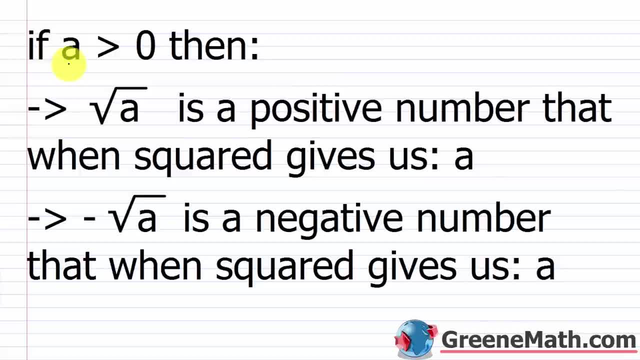 So let's look at kind of a general statement for this. If a is greater than zero. So we know that's a positive value. Then we can say that the square root of 100 is negative 10. So that's a positive number that when squared gives us a. So in other words, if I have the square root of, again, I go back to 225. So this represents a here. So this is a positive number that when squared, when multiplied by itself, gives us this number back. So in this case, this is 15. Because 15 times 15 would give me 225 or that number that's inside of that symbol back. Now we have that negative outside in front of the symbol here. Negative square root of a is a negative number that when squared gives us a. So this is a, the number inside of here. So if I did negative square root of 225, the answer here would be negative 15. So you want to know the two different ways to notate that. Because kind of moving forward on your test, if your teacher says, okay, I want the square root. 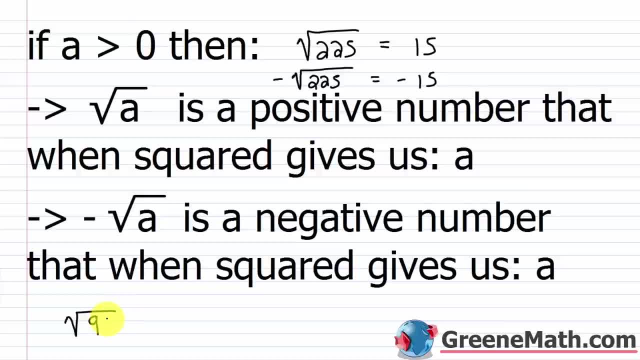 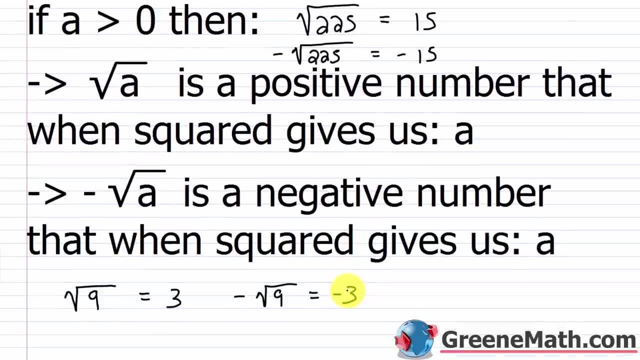 Of let's say the number nine, you have to know that the answer is three, just positive three. If she was to say, I want the negative square root of nine, you have to know that the answer is going to be negative three. And then kind of moving forward as we get higher in math, 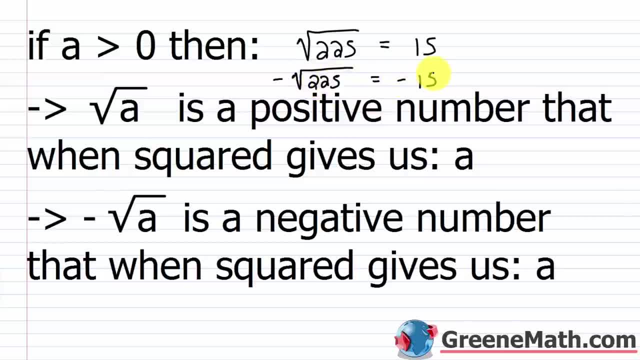 The answer here would be Negative 15.. I want to know the two different ways to notate that Because, kind of moving forward on your test, If your teacher says Okay, I want the square root Of, let's say, The number nine. 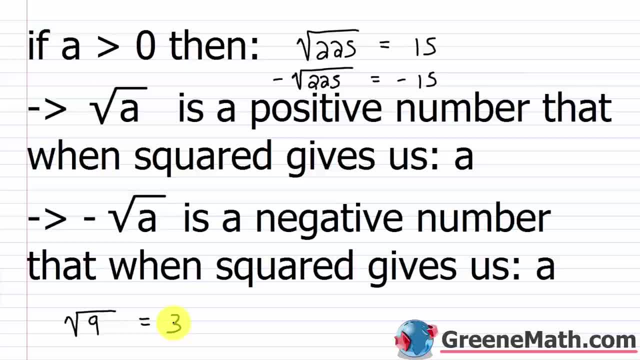 You have to know that the answer is three, Just positive three. If she was to say I want the negative square root of nine, You have to know That the answer is going to be negative three And then kind of moving forward. 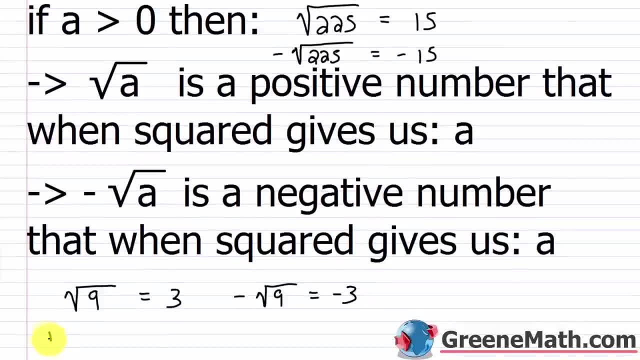 As we get higher in math, You might see them put Or minus The square root of nine And then, in this case, The answer is three, Or it could also be negative. three Because I've accounted for the positive Or principle square root of nine. 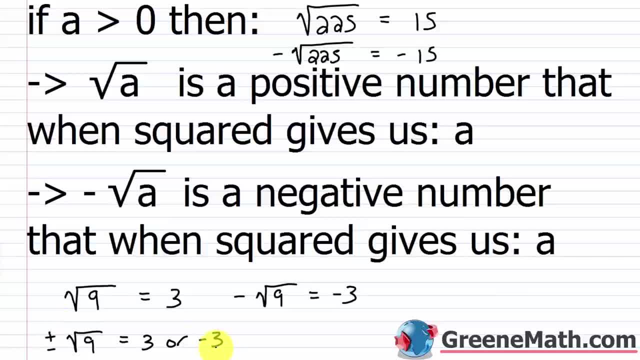 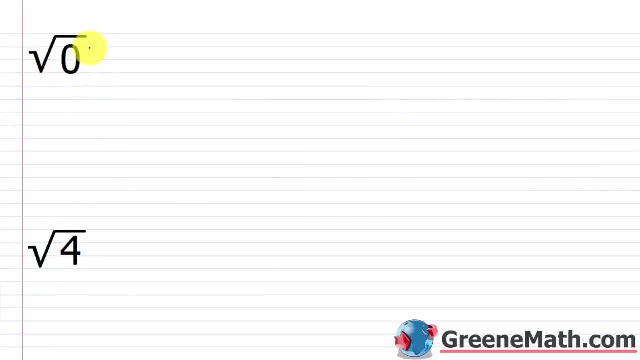 And then also the negative square root of nine. So in that case You get three or negative three. Alright, let's just go through some examples real quick. If I have the square root of zero, Okay, the square root of zero. Zero is not a positive or a negative number. 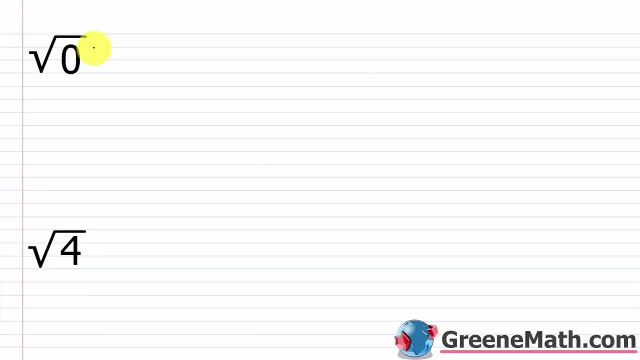 It's just zero. So, in this particular case, What's it going to be equal to? What number multiplied by itself Gives me zero. Well, zero does So. this is an automatic. You see this on your test. You have the square root of zero. 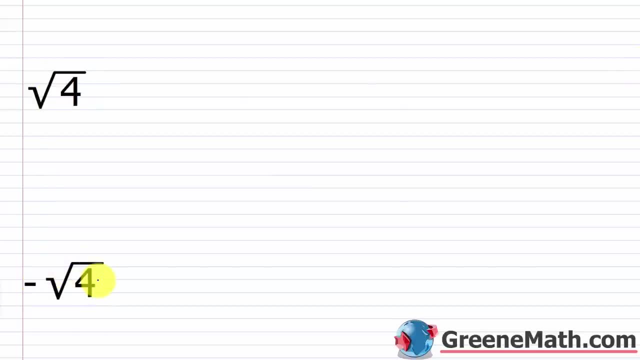 It's just equal to zero. Now the next one. We have the square root of four, And then after that we have the negative square root of four. So the positive or principle square root of four Is what It's two. So what number multiplied by itself? 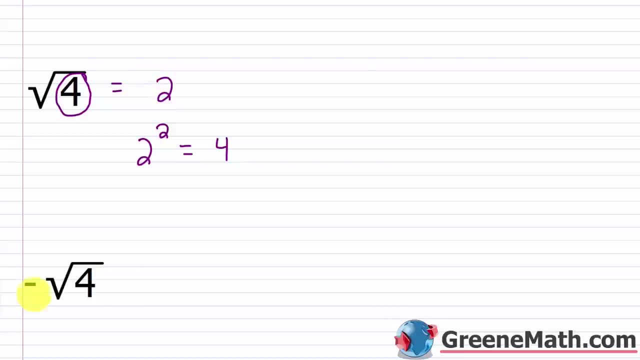 Gives me this: Well, it's two. Two squared is four. Then for this one I have the negative square root of four. So what negative value, When multiplied by itself, is going to give me four? Well, that's negative two. So you can see the difference in the notation. 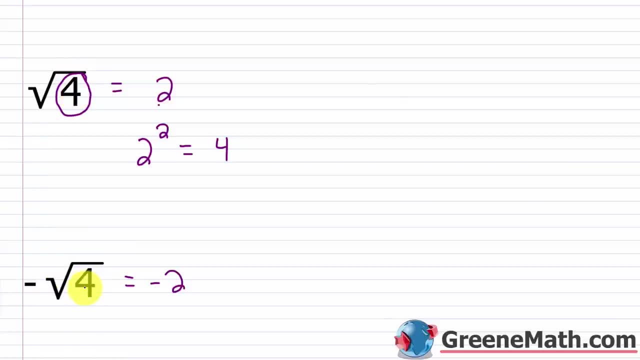 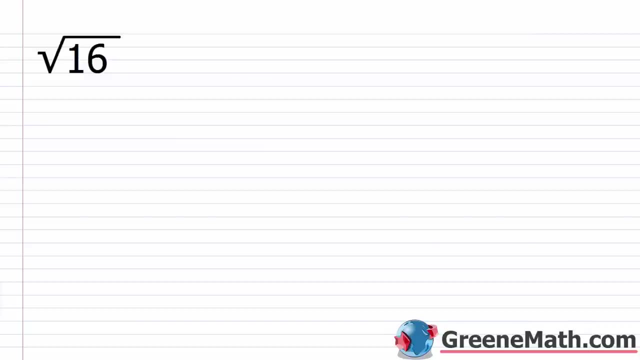 Principle, or positive square root of four, Negative square root of four. So something you really need to pay attention to. Alright, what about the square root of sixteen? Can you think about a number That gives you sixteen Again, if you don't know that off the top of your head? 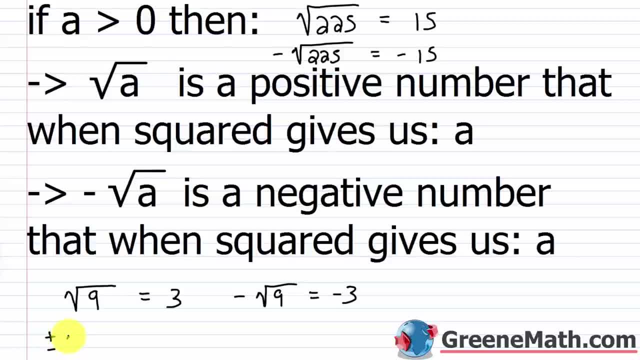 you might see them put plus or minus the square root of nine. And then in this case, the answer is three, or it could also be. Negative three, right? Because I've accounted for the positive or principal square root of nine, and then also the negative square root of nine. So in that case, you get three or negative three. 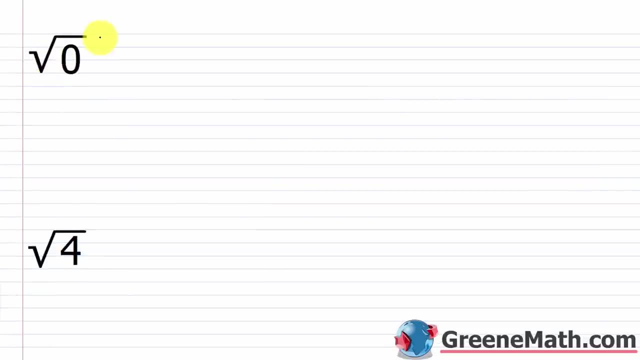 All right, let's just go through some examples real quick. If I have the square root of zero, okay, the square root of zero, zero is not a positive or a negative number. It's just zero. 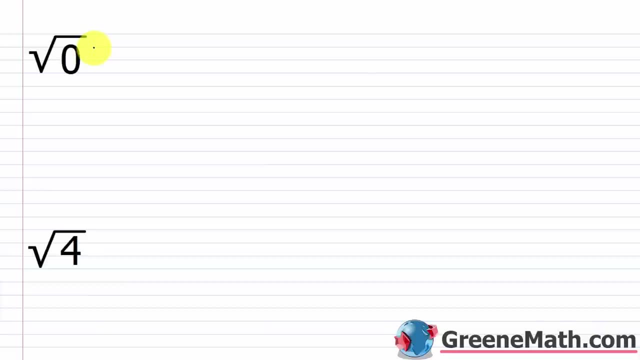 So in this particular case, what's it going to be equal to? What number multiplied by itself gives me zero? Well, zero does. 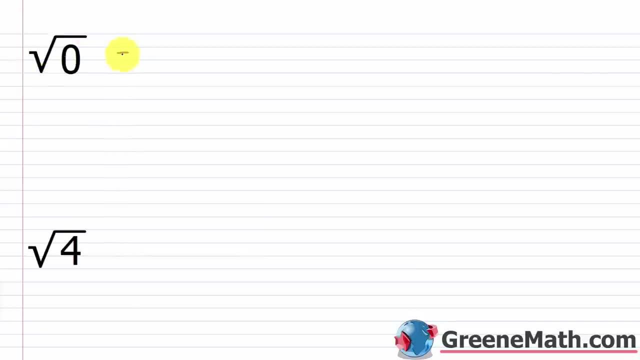 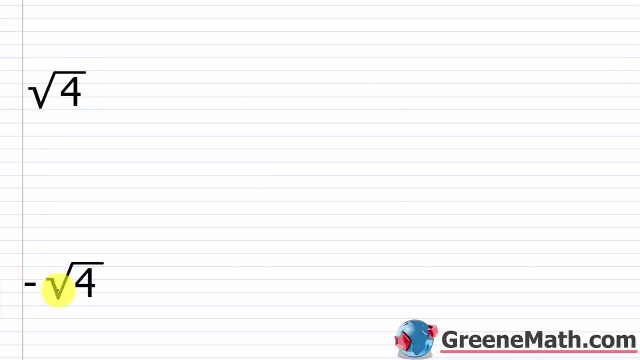 It's an automatic. You see this on your test. You have the square root of zero. It's just equal to zero. Now the next one, we have the square root of four. And then after that, we have the negative 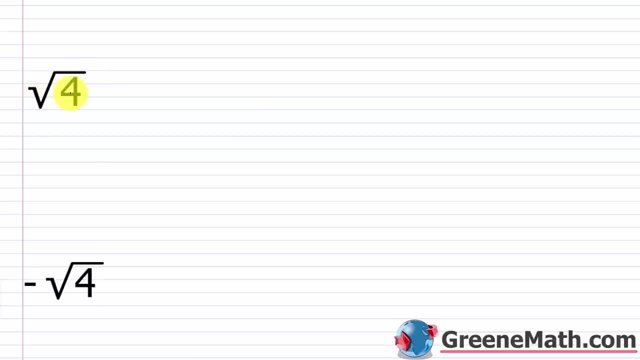 square root of four. So the positive or principal square root of four is what? It's two, right? Because two squared is going to give me four, right? What number multiplied by itself gives me this? Well, it's two, right? Two squared is four. Then for this one, I have the negative square root of four. 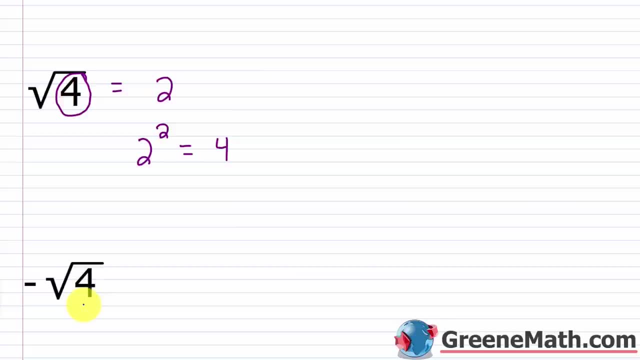 So what negative value when multiplied by itself is going to give me four? Well, that's negative two. 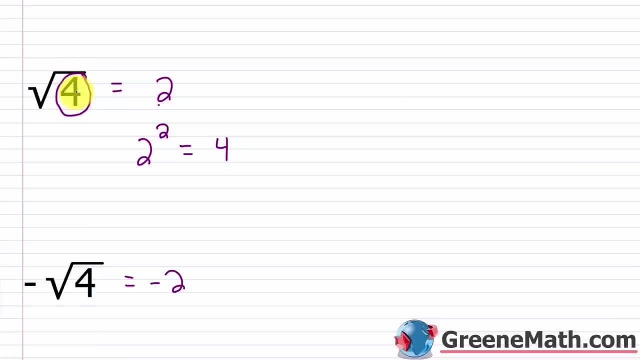 So you can see the difference in the notation. Principal or positive square root of four, negative square root of four. So something you really need to pay attention to. 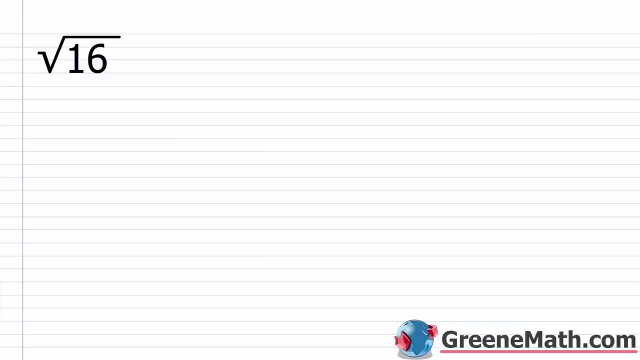 All right, what about the square root of 16? Can you think about a number that when multiplied by itself gives you 16? Again, if you don't know that off the top of your head, always just build a factor tree. So I could say, okay, 16 is what? A lot of you right away know it's four times four. 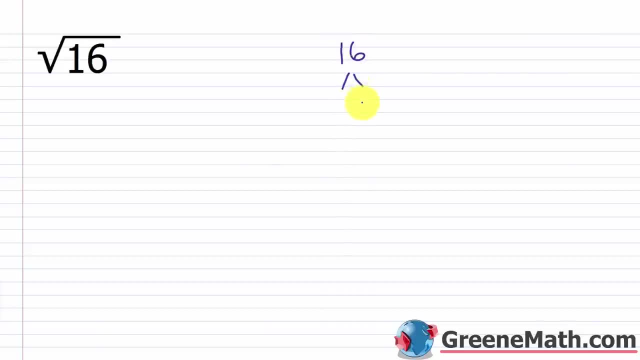 Always just build a factor tree So I can say, okay, sixteen is one. A lot of you right away know it's four times four. But let's say you did. Let's say you start out with eight times two. You know that two is prime. 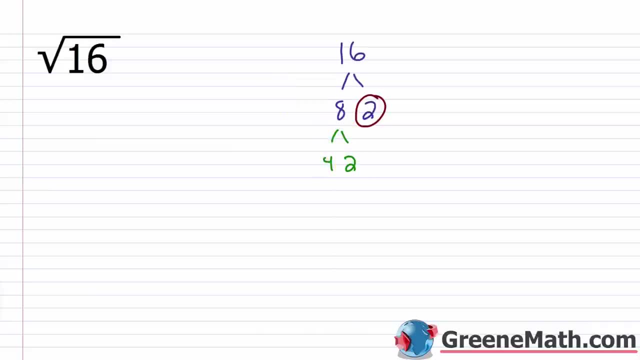 And for eight. You know that's four times two And you know two is prime. At that point you could stop. You could say: okay, two times two is four, You'd have four times four, This is two times two. So now you see. 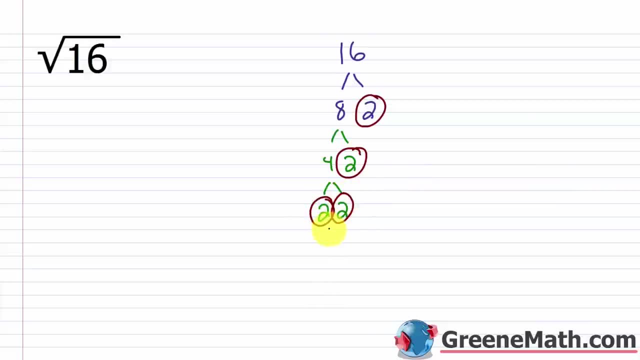 That you have what? Two times two or four. This is four times Two times two or four. Alright, so four times four, Which is sixteen, So a number that is multiplied by itself. That gives me: this is my answer. So the square root of sixteen is four. 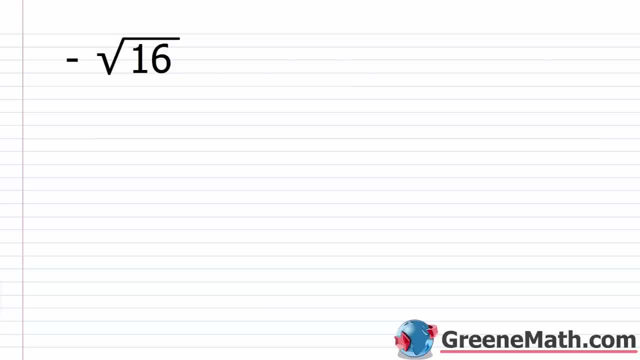 And then, what about the negative Square root of sixteen? Well, again, what negative number When multiplied by itself? Well, negative four. Negative four times negative four Is positive sixteen. Alright, what about the square root of four hundred? Well, a lot of you are not going to know. 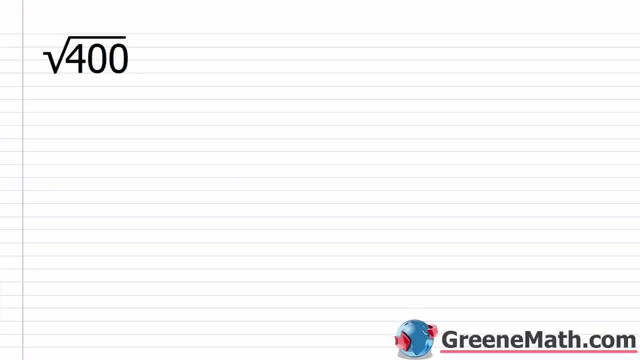 What number multiplied by itself gives you four hundred. So let's just start out with A factor tree. So four hundred, I know it ends in zero, so it's divisible by ten. So this would be what Forty times ten, And ten I can break down into five times two. 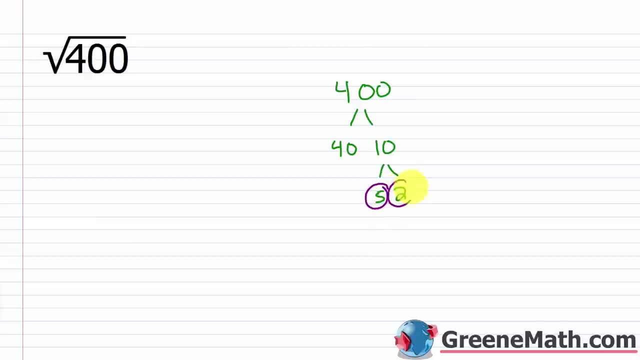 Those are each going to be prime. So let's circle those Then for forty. I can break that down into ten times four, And ten is five times two, And four is two times two. Let's circle all these. So what do I see here? 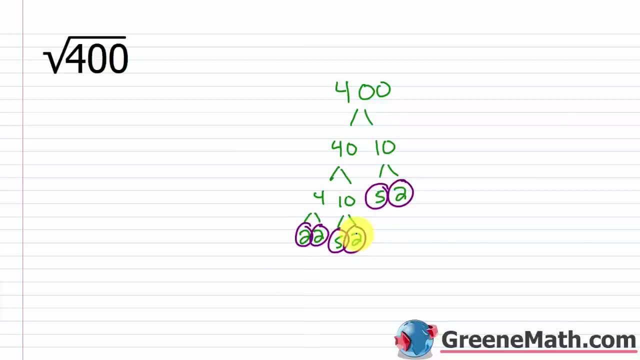 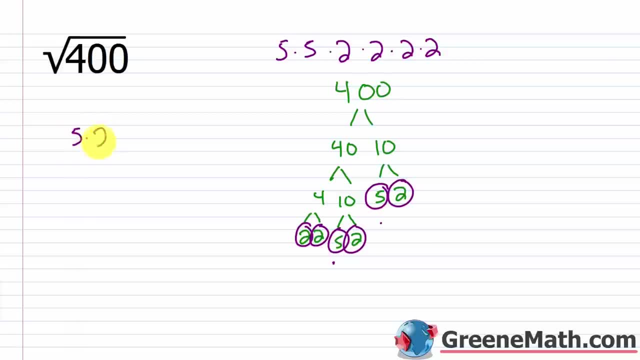 Five Times two times two Times Five times two times two, Or five times four, Which is twenty Times twenty. Twenty times twenty is four hundred. So that's your answer, And sometimes, when you don't know, these off the top of your head. 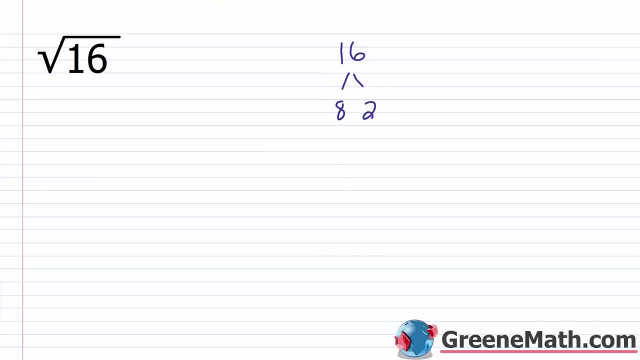 But let's say you did. Let's say you start out with eight times two. You know that two is prime. And for eight, you know that's four times two. And you know two is prime. At that point, you could stop. You say, okay, two times two is four. You'd have four times four. But let's say you just kept going. Okay, we keep going. This is two times two. So now you see that you have what? Two times two or four. This is four times two times two or four. 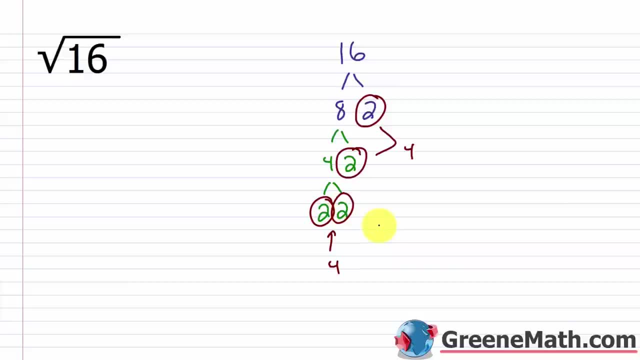 So four times four, which is 16. So a number that is multiplied by itself that gives me this is my answer. So the square root of 16 is four. And then what about the negative square root of 16? 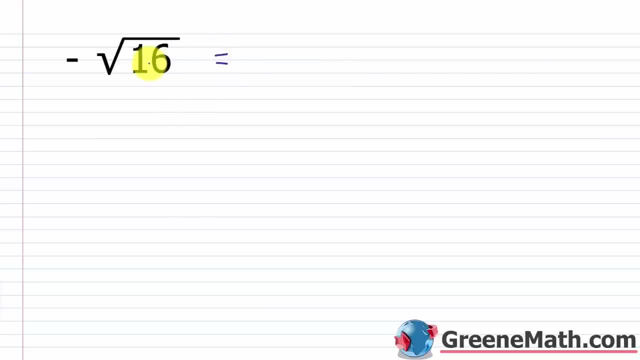 Well, again, what negative number when multiplied by itself is going to give me 16? Well, negative four. Negative four times negative four is positive 16. All right, what about the 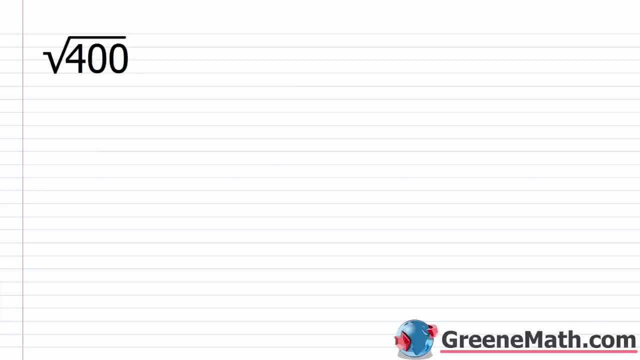 square root of 400? Well, a lot of you are not going to know what number multiplied by itself gives you 400. So what about the square root of 400? Well, a lot of you are not going to know what 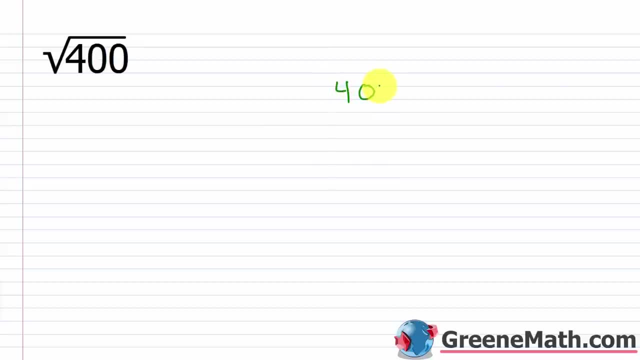 So let's just start out with a factor tree. So 400, I know it ends in zero, so it's divisible by 10. So this would be what? 40, 40 times 10. 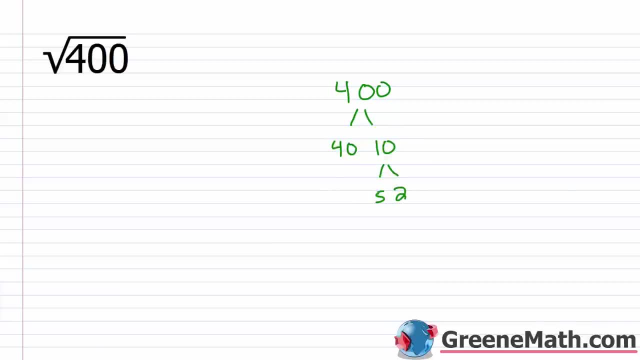 And 10, I can break down into five times two. Those are each going to be prime. So let's circle those. 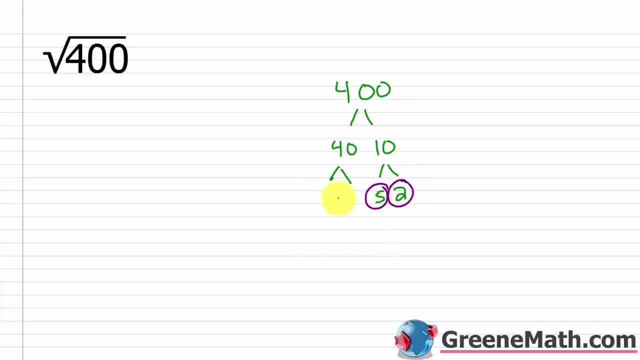 Then for 40, I can break that down into 10 times four. And 10 is five times two. And four is two times two. So let's circle all these. 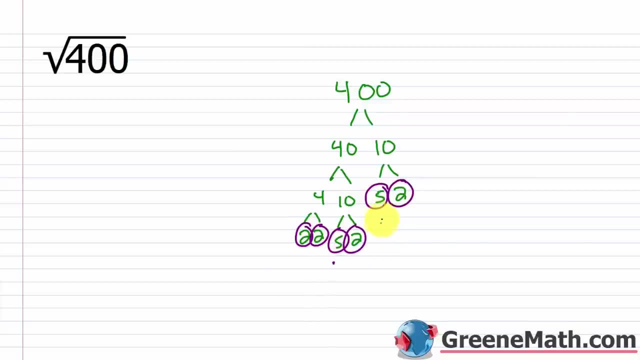 So what do I see here? I've got one, two fives. 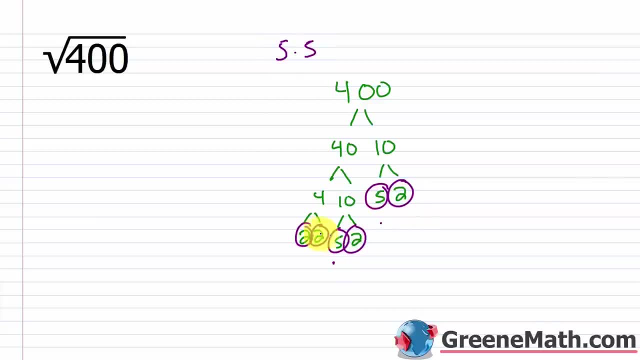 So five times five. And I've got one, two, three, four twos. 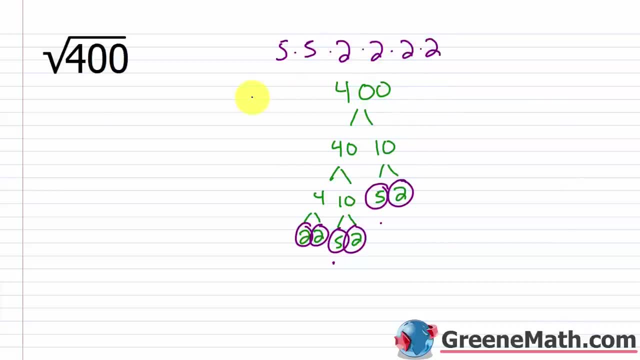 Well, what I can do is I can write this as what? Five times two, times two, times five, times two, times two. 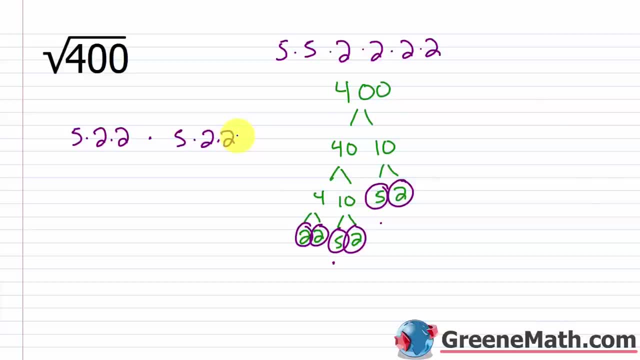 Or what I can do is I can write this as what? 5 times 4, which is 20, times 20. 20 times 20 is 400. So that's your answer. And sometimes when 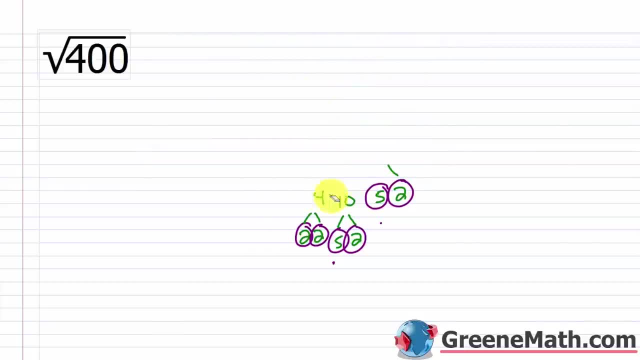 you don't know these off the top of your head, you've got to do a little bit of work. But pretty much in Algebra 1, they're going to keep giving you kind of the same ones over and over again. 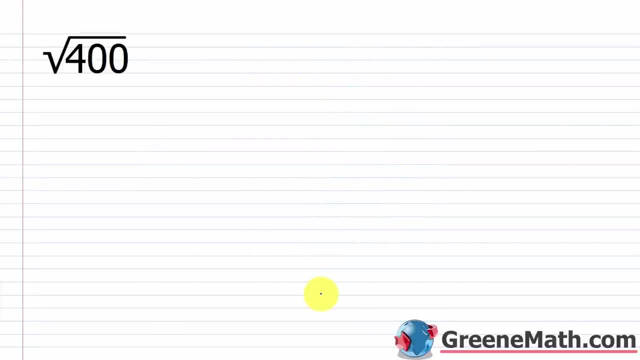 You've got to do a little bit of work, But pretty much in algebra one They're going to keep giving you kind of the same ones over and over again And you'll memorize them very, very quickly. You also have something on your calculator. 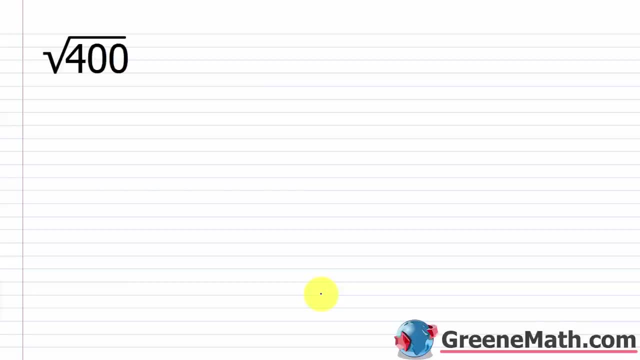 If you're allowed to use it, Known as a square root key, Right? so you type in a number And then hit square root And then it's going to give that to you automatically. So the square root of four hundred would be twenty. 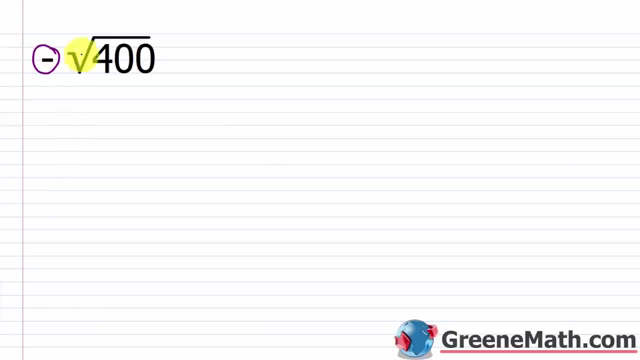 Now, Again, we have the negative square root of four hundred, And so this is what This is: negative twenty, Since negative twenty times negative twenty Would give you four hundred. Alright, so we're also going to see this with fractions As well. 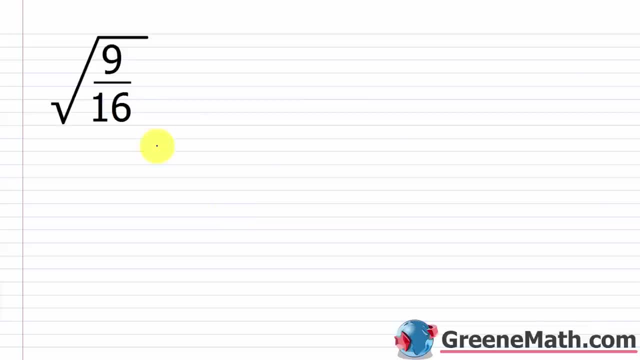 So we have the square root of nine sixteenths. So just think about what fraction Times itself Would give me nine sixteenths. We'll just break up the numerator and denominator Kind of separately. in your head, What number? 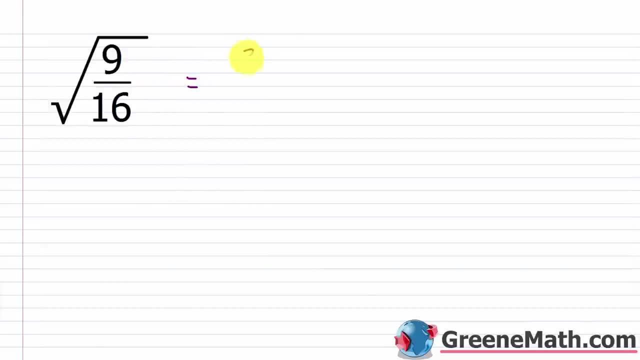 Multiplied by itself, would give me nine. We know that would be three. Then what number multiplied by itself, Would give me sixteen. We know that would be four And you can check it. Would three. fourths, Would give me nine. sixteenths, 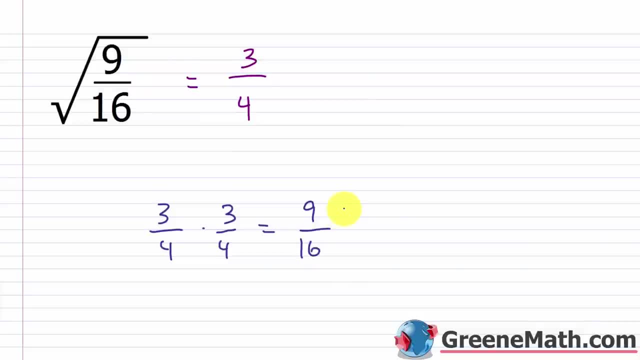 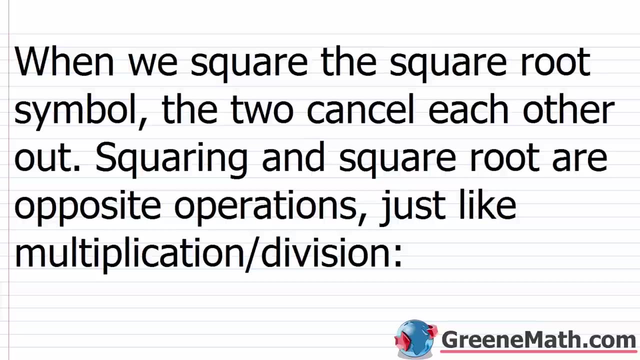 Three times three is nine, Four times four is sixteen. So, yeah, that does check out Alright. so let's talk about something that is going to come up Kind of as we move forward. When we square the square root symbol, The two cancel each other out. 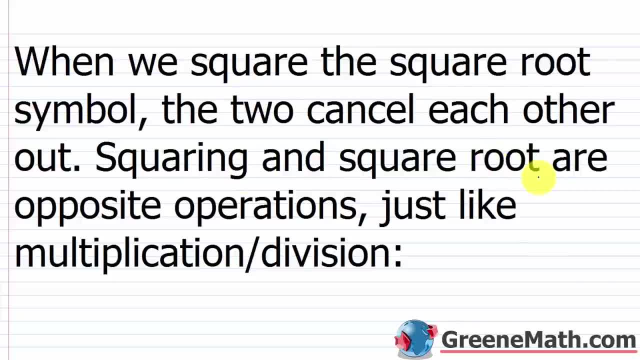 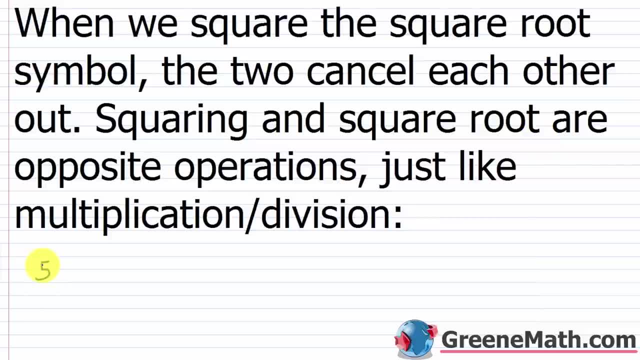 So squaring and square root Are opposite operations, Just like multiplication and division. So, in other words, if I had Something like five, I start with that And then I multiply by three. Well, what's going to happen? I'm going to end up with five again. 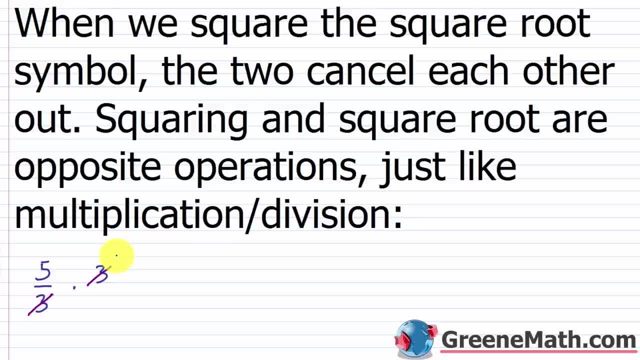 Because this operation, The division, cancels with the multiplication. If I divide by three But then I multiply by three, I just start out with that original number five, So this just equals five. It's going to be the same thing If I started out with, let's say, five. 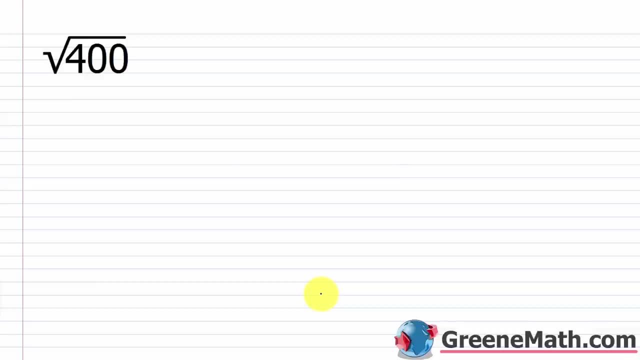 So you'll memorize them very, very quickly. You also have something on your calculator, if you're allowed to use it, known as a square root key, right? So you type in a number and then hit square root, and then it's going to give that to you automatically. So the square root of 400 would be 20. Now, again, we have the negative square root of 400. And so this is what? This 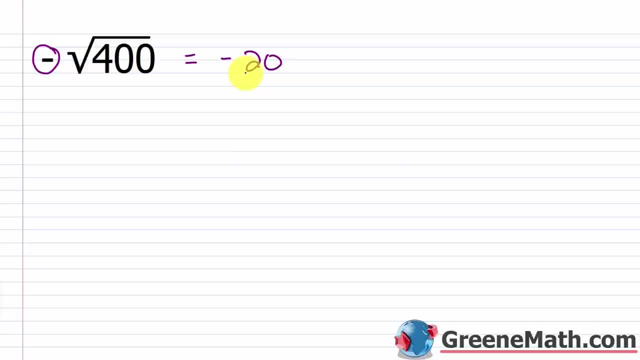 is negative 20, since negative 20 times negative 20 would give you 400. All right, so we're also going to see this with fractions as well. So we have the square root of 9 16ths. So just think 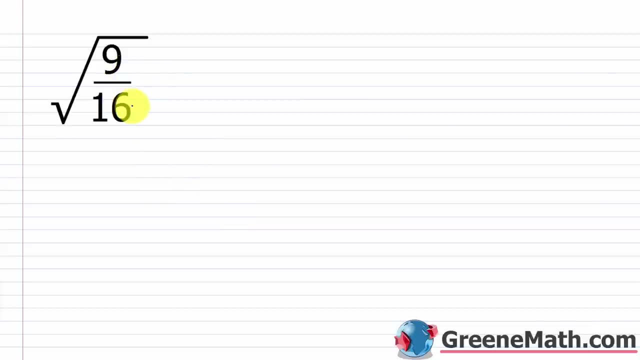 about what fraction times itself would give me 9 16ths. Well, just break up the numerator and denominator kind of separately in your head. What number multiplied by itself would give me 9? We know that would be 3. Then what number multiplied by 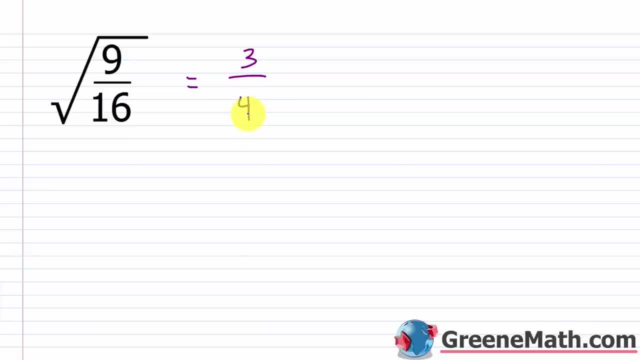 itself would give me 16? We know that would be 4. And you can check it. Would 3 4ths times 3 4ths give me 9 16ths? 3 times 3 is 9. 4 times 4 is 16. So yeah, that does check out. All right, 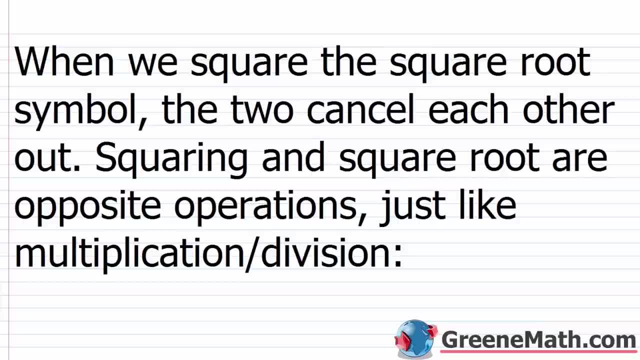 let's talk about something that is going to come up kind of as we move forward. 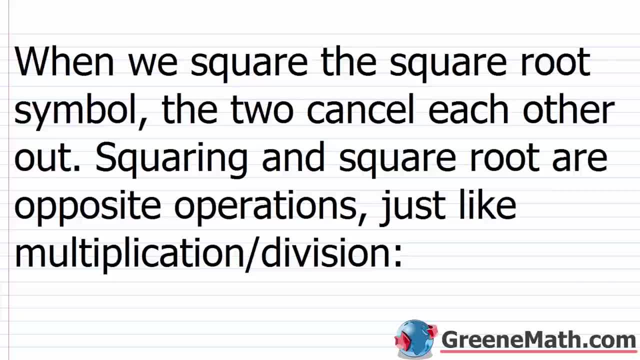 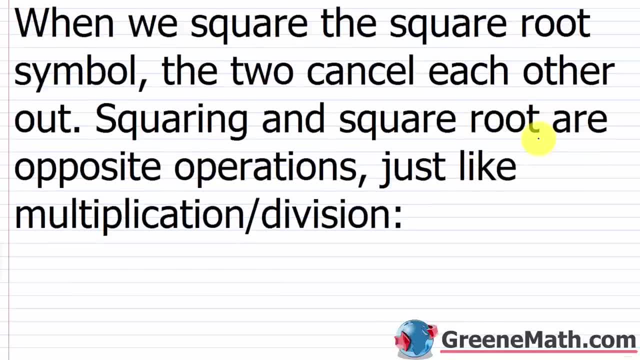 When we square the square root symbol, the two cancel each other out. So squaring and square root are opposite operations, just like multiplication and division. So in other words, if I had something like 5, I start with that. Let's say I divide 5 by 3. And then I multiply by 3. Well, what's going to happen? I'm going to end up with 5 again, right? Because this operation, the division, cancels with the multiplication, right? If I divide by 3, but then I multiply, 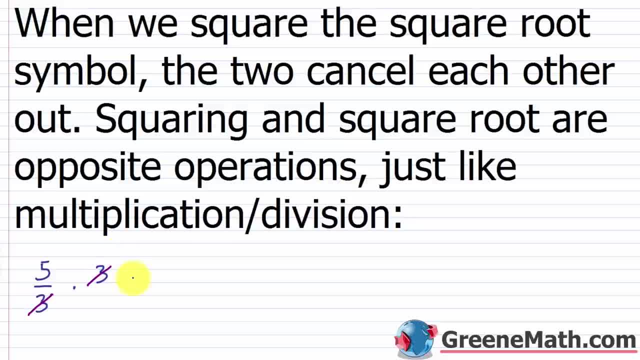 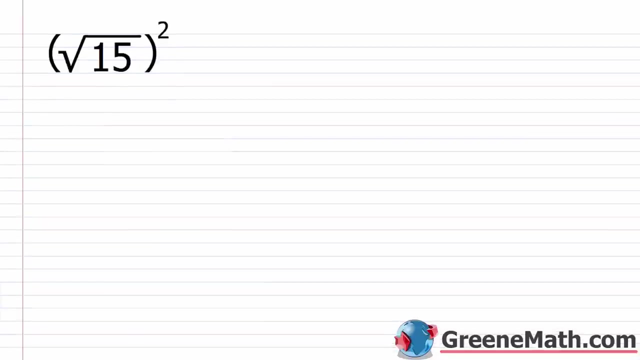 I just start out with that original number 5, right? So this just equals 5. It's going to be the same thing. If I started out with, let's say, 5. And let's say I have 5. And I square 5. But then I take the square root, I'm going to end up with 5 again, right? 5 squared is what? It's 5 times 5. That's 25. And then if I took 25, and I took the square root of it, I'm going to end up with 5 again, right? So it's just like multiplication and division. They're opposite operations. So we have here the square root of 15 that's squared. So in other words, I start out with 15, I take the square root of it, but then I square it. So it's like, I can cancel this and this, and I'm just left with this, right? And another way to show that is just to say, okay, 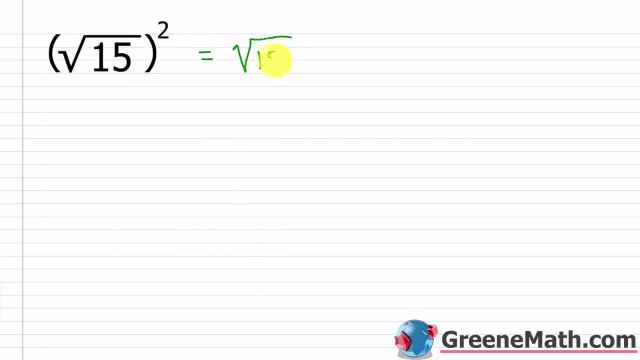 well, what I have here is I have the square root of 15 times the square root of 15. So whatever 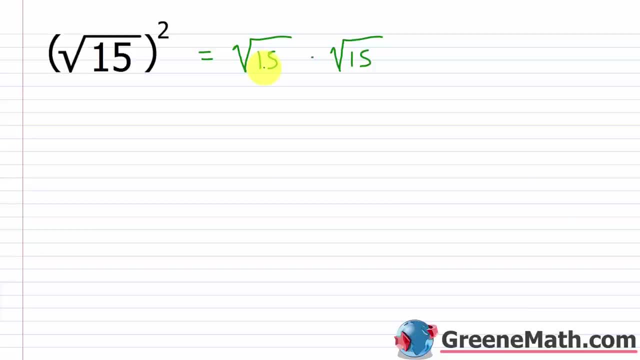 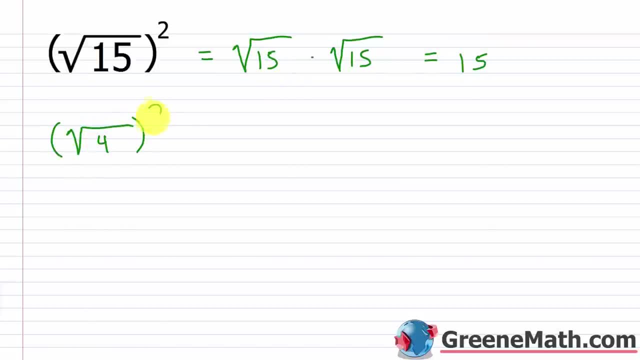 had something like the square root of 4 squared. So writing this the same way, this is square root of 4 times square root of 4. Does this equal 4? We know that the square root of 4 is 2. So what is 2 times 2? Well, 2 times 2 is 4, right? So that's where this comes from. Kind of the shortcut to 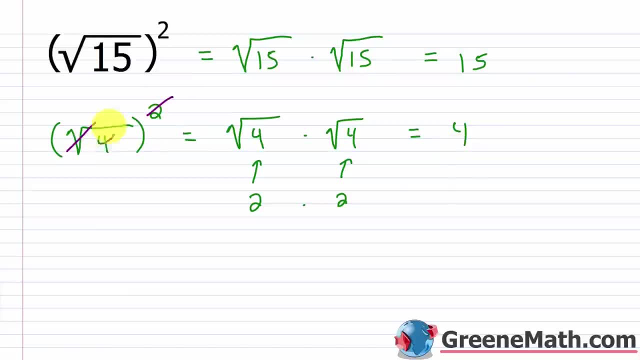 this is just to say, okay, I'm going to take the square root of 4 times the square root of 4. So this is going to cancel with this, and I just have this. So what if I had the negative square 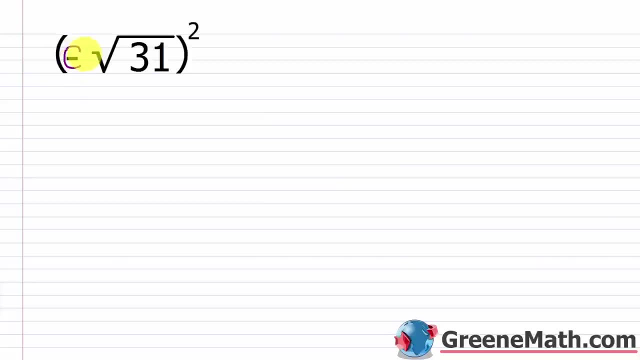 root of 31 squared? So if I square a negative, right, you think about that as just negative 1. 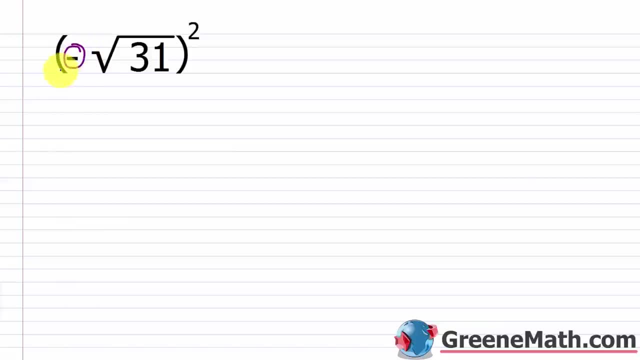 Negative 1 times negative 1 is 1. So this and the square root are going to cancel, and I'm going to be left with 31. Again, if you want to think about this in a different way, think about if you had negative square root of 31 multiplied by negative square root of 31. Negative times negative is positive, of course. Square root of 31 times the square root of 31 is just 31. All right, 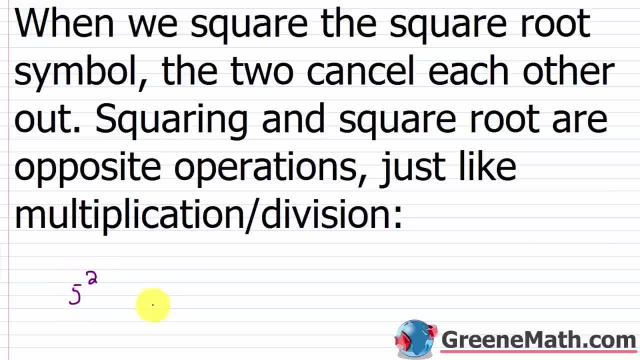 And let's say I have five And I square five, But then I take the square root. I'm going to end up with five again. So that's five times five, That's twenty five. And then if I took twenty five, 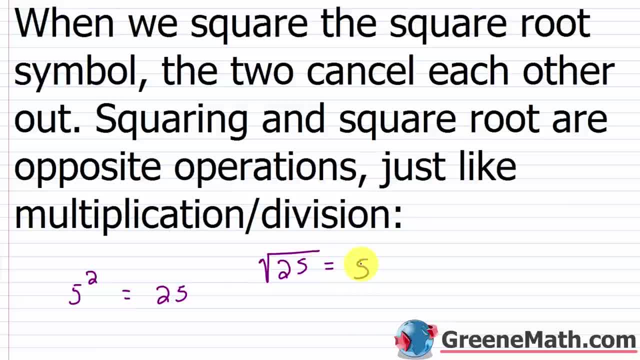 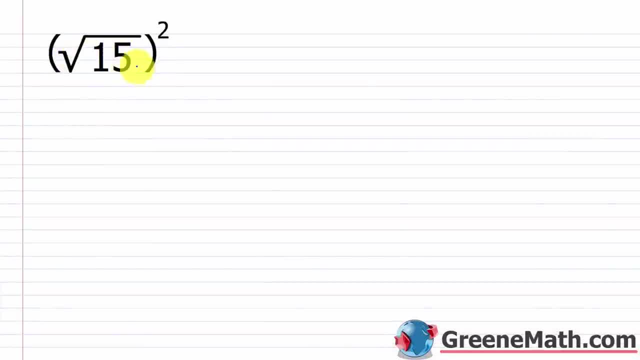 And I took the square root of it. I'm going to end up with five again. So it's just like multiplication and division. They're opposite operations. So we have here the square root of fifteen. That's squared. So in other words, 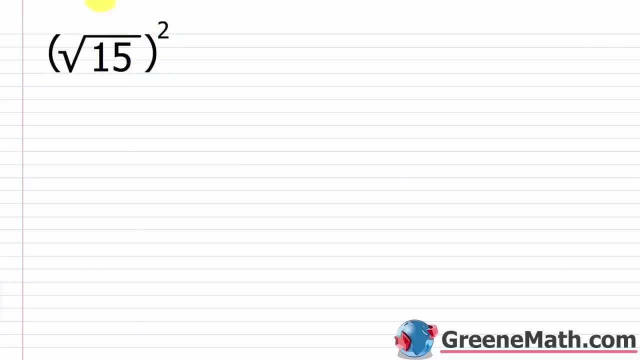 I start out with fifteen. I take the square root of it, But then I square it, So it's like I can cancel this and this And I'm just left with this. It's just to say What I have here is I have the square root of fifteen. 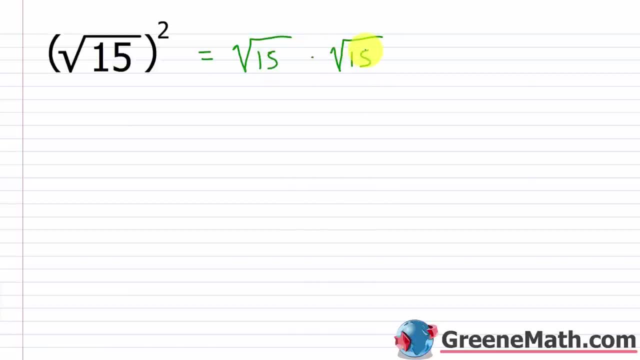 Times the square root of fifteen. So whatever number it is For fifteen, That multiplied by itself Gives me fifteen. It's multiplied by that number, So I would just get fifteen Right. As an easier example, Let's say I had something like the square root of four. 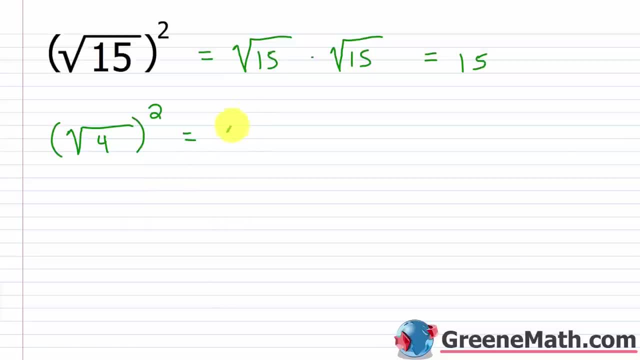 Squared. So, writing this the same way: Square root of four times square root of four, Does this equal four? We know that the square root of four is two. So what is two times two? Well, two times two is four. So that's where this comes from. 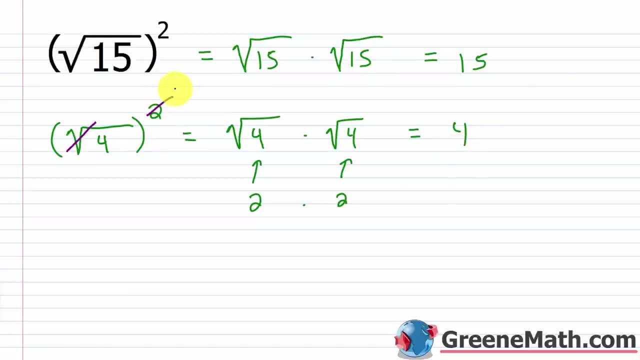 Kind of the shortcut to this is just to say: Okay, well, this is going to cancel with this And I just have this. So what if I had the negative square root of thirty one squared? So if I square a negative Right, You think about that as just negative one. 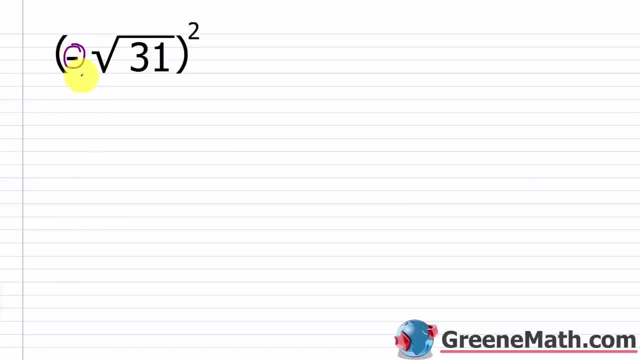 Negative one times negative, one is one. So this and the square root Are going to cancel And I'm going to be left with thirty one Again. if you want to think about this in a different way, Think about if you had negative. 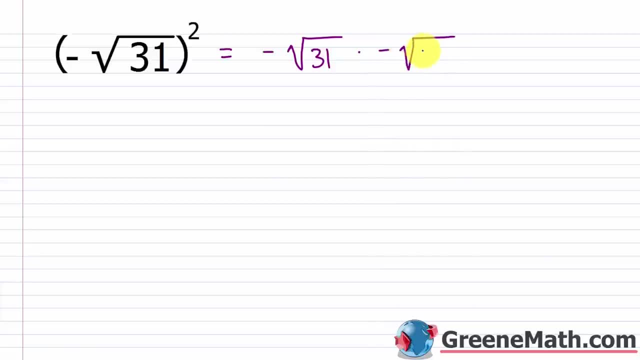 Square root of thirty one Multiplied by negative Square root of thirty one. Negative times negative is positive, of course. Square root of thirty one times the square root of thirty one Is just thirty one. Alright, so this one is a bit more complex. 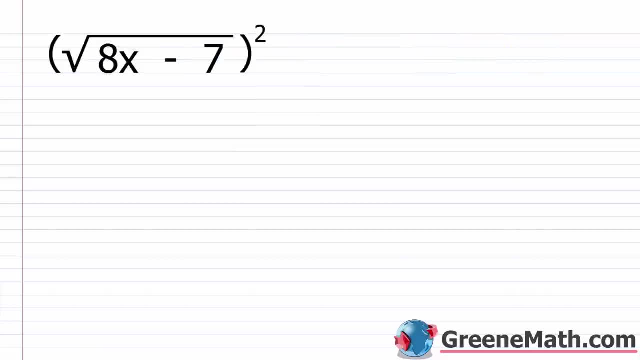 so this one's a bit more complex, but we follow the same logic. So we have the square root of 8x minus 7, and this is squared. So this is going to cancel with this, and I'll just have what's inside, 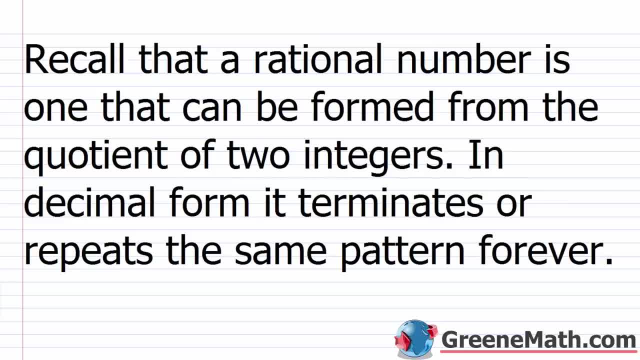 which is 8x minus 7. All right, let's talk a little bit more about rational numbers and irrational numbers, which we've kind of covered before, but I want to make sure that you guys have kind of a strong foundation in this before we get to Algebra 2 and we really start knocking some numbers around. So I want you to recall that a rational number, let me just highlight that, 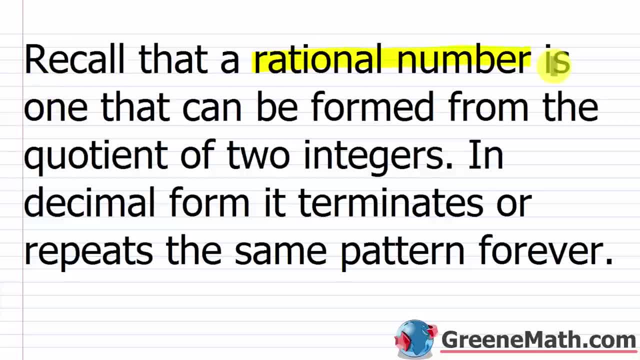 a rational number is one that can be formed from the quotient of two integers. In decimal form, it's going to terminate, okay, or it's going to repeat the same pattern forever. So you've seen something like 21.3, and we put a bar over the 3 because the 3 repeats forever. That is a rational number. Or you've seen something like, you know, let's say you have 0.687, 687, 687, you know, where the 6, the 8, and the 7 repeat forever, right? And we could erase this and just put a 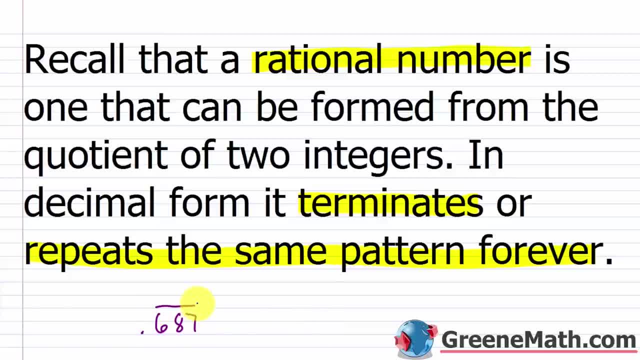 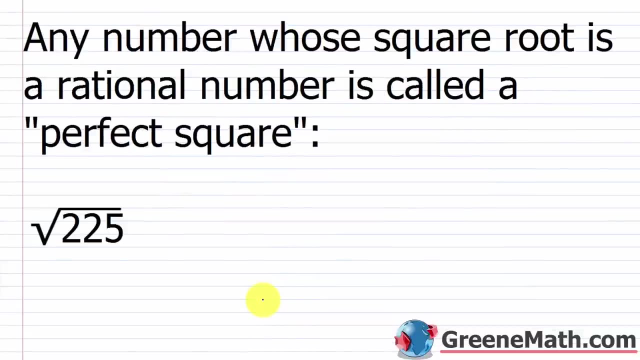 bar over this. So that pattern repeats forever. Or it terminates. So you might just get 0. 6, 8, 2, 5, 9, 1, and it stops. Those are rational numbers, right? You can always form these from the quotient of two integers. So I should be able to say this is, let's say, 28 over 3, one integer over another. So any number whose square root is a rational number is called a 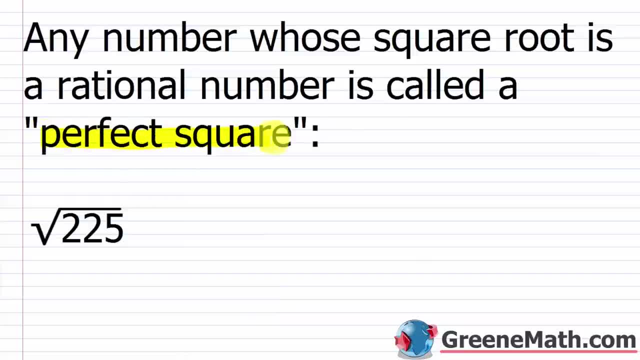 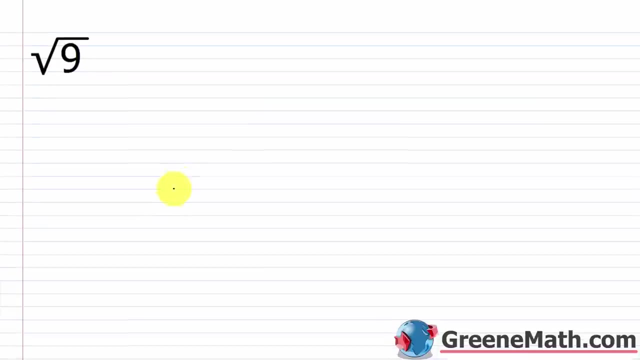 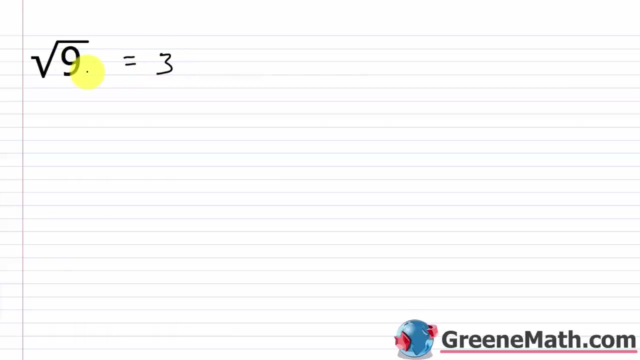 perfect square, a perfect square. You're going to hear me talk about that all the time. You've also talked about polynomials. I refer to a perfect square trinomial. So to go back to an example that we already know, the square root of 225 is what? It's 15. 15 is a rational number. So therefore, 225 is a perfect square. And then there's another example that we already know. The square root of 9 is what? It's 3. So 3 is a rational number. So therefore, 9 is a perfect square. What about the square root of 1 fourth? Well, this is what? 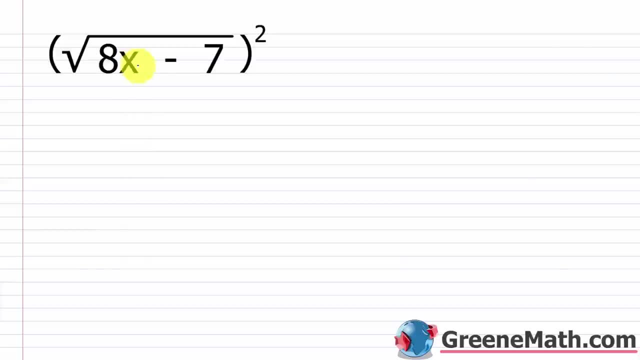 But we follow the same logic. So we have the square root of eight x minus seven And this is squared. So this is going to cancel with this And I'll just have what's inside, Which is eight x minus seven. Alright, 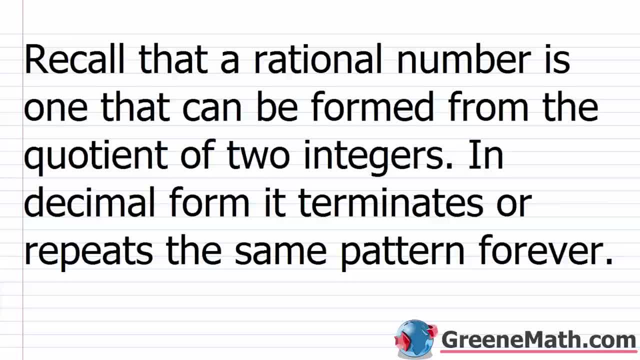 Let's talk a little bit more about Rational numbers and irrational numbers, Which we've kind of covered before. But I want to make sure that you have Kind of a strong foundation in this Before we get to algebra two And we really start knocking some numbers around. 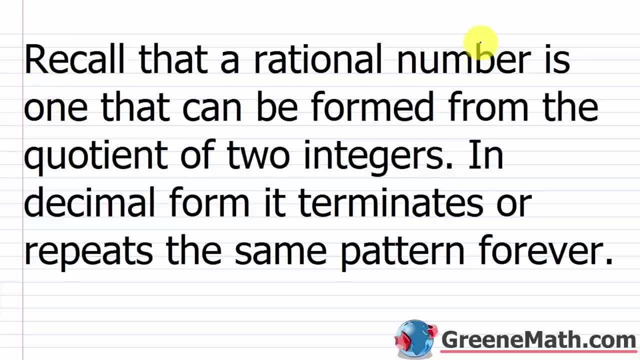 So I want you to recall That a rational number- Let me just highlight that A rational number- Is formed from the quotient Of two integers In decimal form. It's going to terminate Or it's going to repeat The same pattern forever. 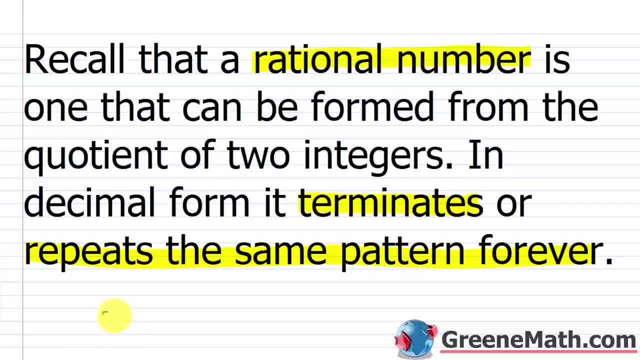 So you've seen examples Where you get something like Twenty one point three And we put a bar over the three Because the three repeats forever. That is a rational number. Or you've seen something like You know. let's say you have 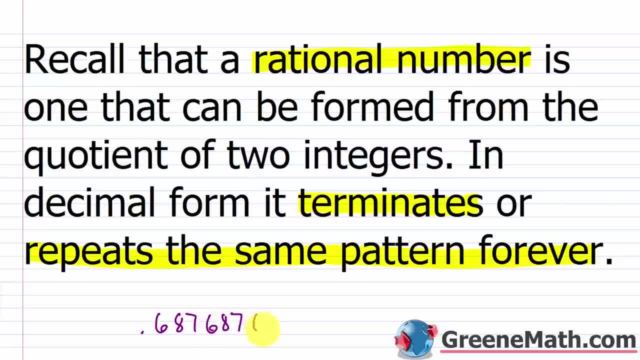 Point six, eight, seven, Six, eight, seven. You know where the six, The eight and the seven repeat forever And we can erase this and just put a bar over this So that pattern repeats forever Or It terminates. So you might just get point six, eight, two. 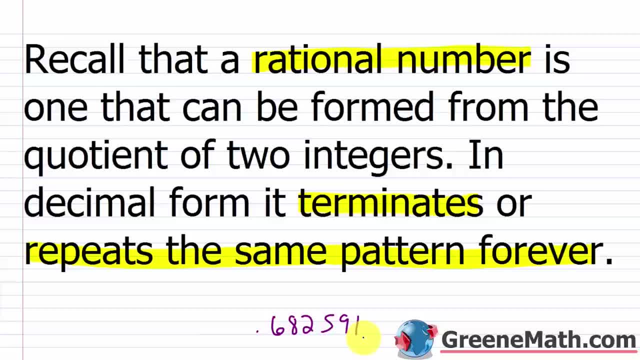 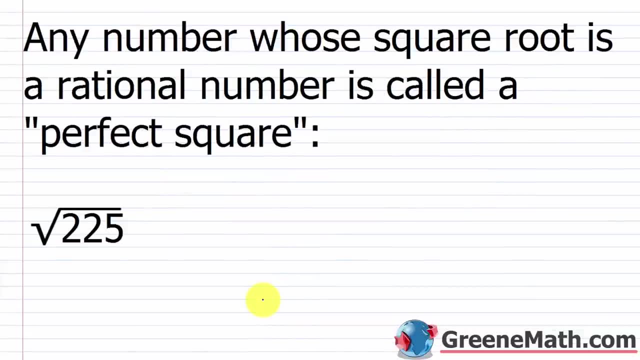 Five, nine, one, And it stops. Those are rational numbers. You can always form these From the quotient of two integers. So I should be able to say Eight over three, One integer over another. So any number Whose square root is a rational number. 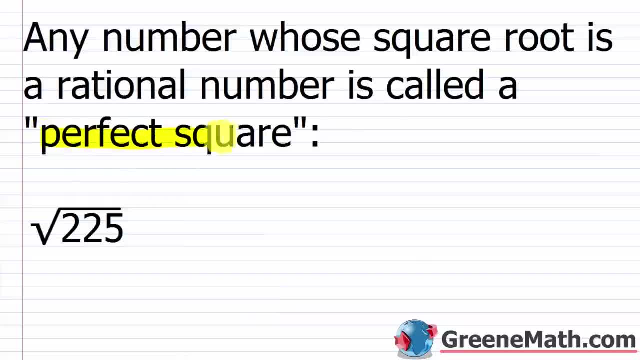 Is called a perfect square. A perfect square. You're going to hear me talk about that all the time. You've also heard me talk about this When we were talking about polynomials. I refer to a perfect square, trinomial. So, to go back to an example that we already know, 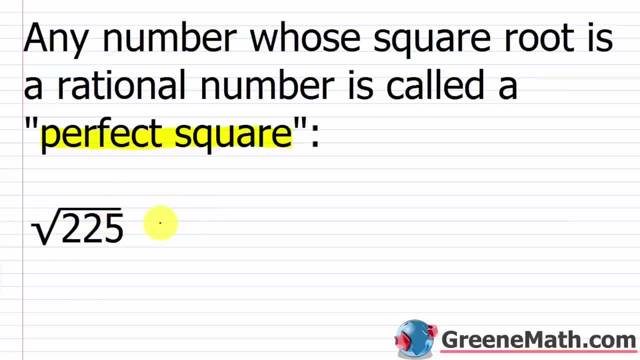 The square root of two hundred twenty five Is what It's fifteen. Fifteen is a rational number, And twenty five is a perfect square. And then there's another example that we already know: The square root of nine is what It's three. 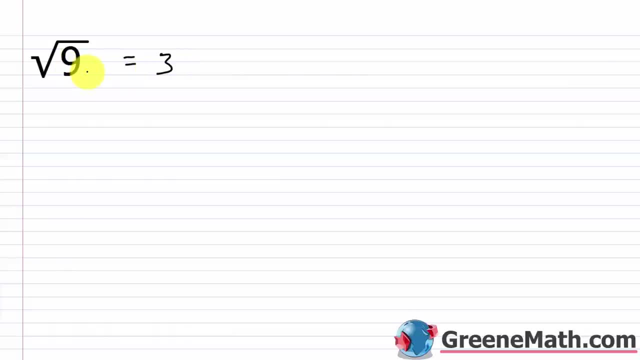 So three is a rational number. So therefore, nine is a perfect square. What about the square root of one? fourth? Well, this is what Square root of one. If I think about, what times? what would give me one? It's one. What times what would give me four? 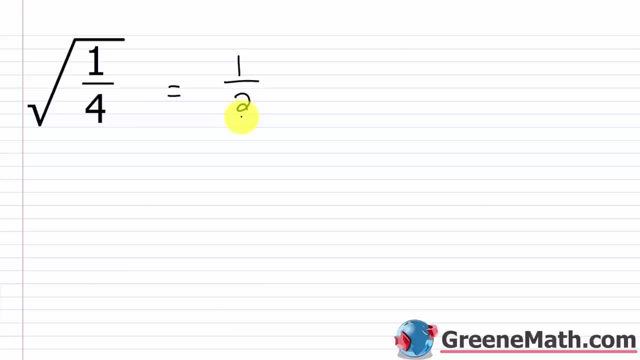 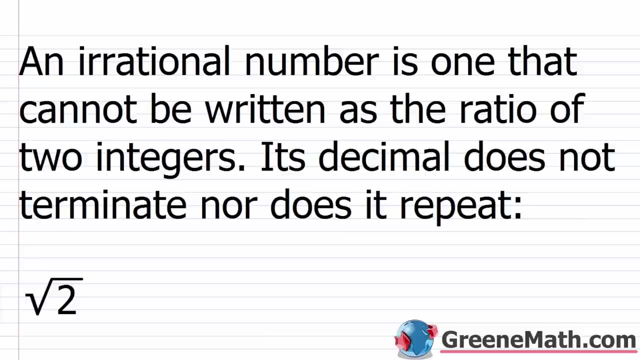 It's two, So the square root of one fourth is one half, And so, therefore, Is a perfect square. Now let's talk a little bit about irrational numbers. So an irrational number Is one that cannot be written As the ratio of two integers. 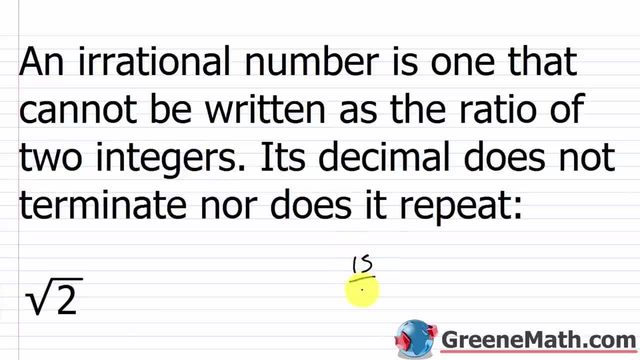 So I can't say This is fifteen over four, For example. I can't do that with an irrational number. There are no two integers that I can put over each other To give me That irrational number, So it's decimal does not terminate. 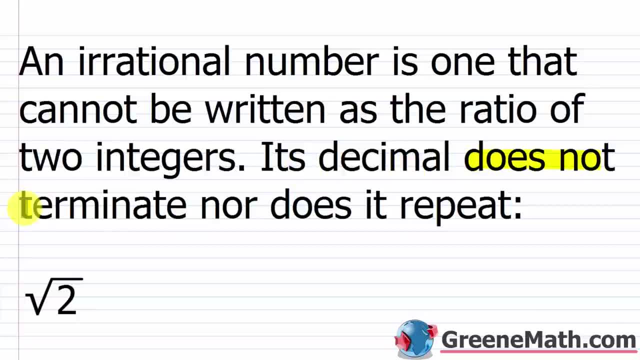 It does not Terminate, Nor does it repeat: Okay, So something like the square root of two. You cannot find two integers that you can put over each other. That would give you The square root of two If you type this into a calculator. 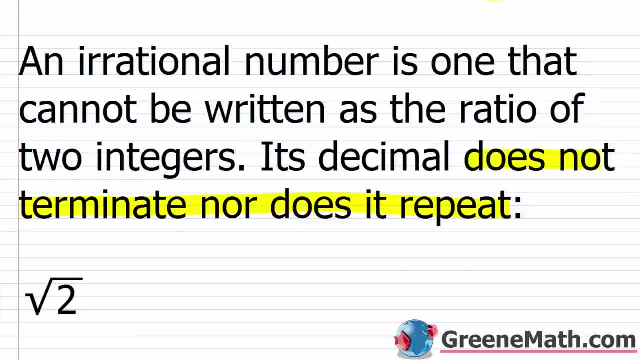 You're not going to get an exact value. Your calculator is either going to round Or it's going to truncate And it's going to give you an estimate for it, But not an exact value, And usually We'll say: this is approximately equal to. 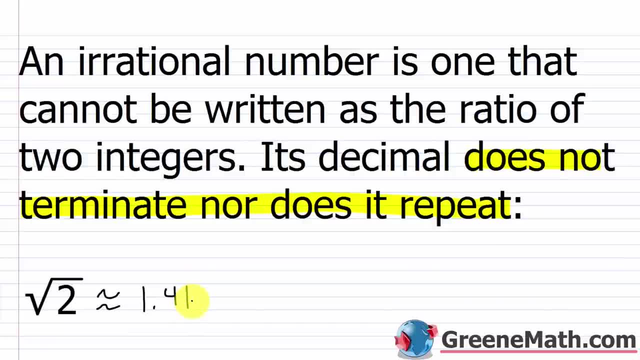 One point four, one Four, two, one Three, five, six, two. But if you type it up on a calculator- And I just typed it up on mine- I get one point four, one Four, two, one Three, five, six, two. So after that, 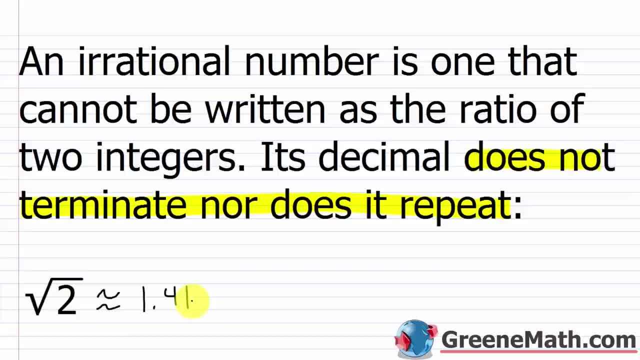 Final digit that you get, Realize that it continues forever And ever and ever, And it's not going to terminate Or repeat the same pattern. So that's the problem with an irrational number. We talked about this before When we talked about direct variation. 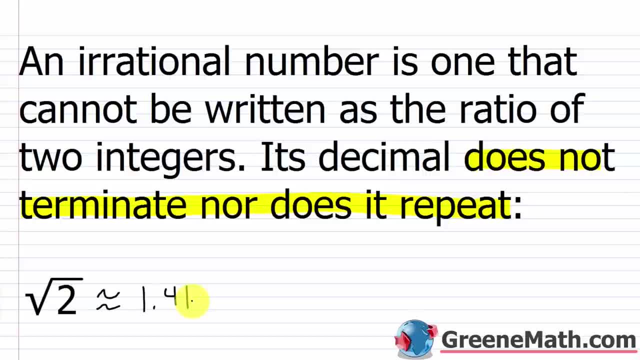 And I gave you an example where, In the Hollywood movie The Life of Pi, This guy, when he was a child, Is on a blackboard And he's reciting all these digits of pi And you can go on a computer And go into Google. 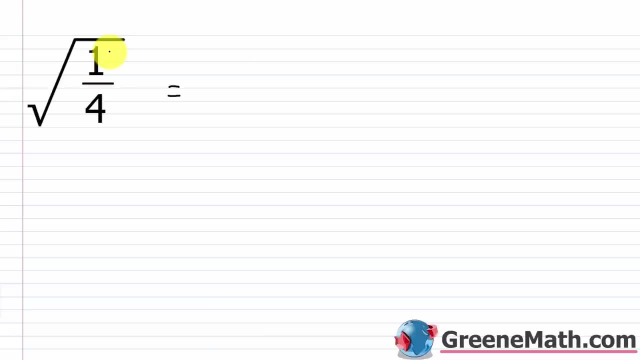 Square root of 1, if I think about what times what would give me 1, it's 1. What times what would give me 4? It's 2. So the square root of 1 fourth is 1 half. And so therefore, 1 fourth is a perfect 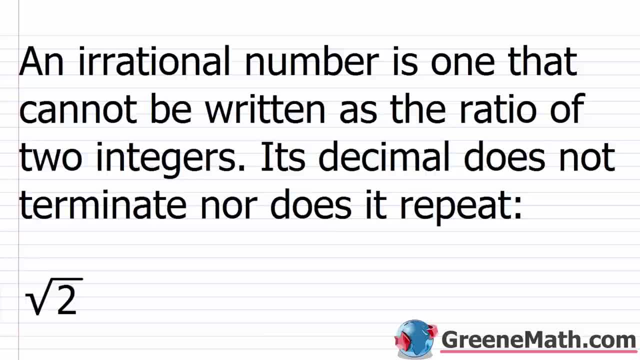 square. All right, now let's talk a little bit about irrational numbers. So an irrational number is one that cannot be written as the ratio of two integers. So I can't say, OK, this is 15 over 4, for example. I can't do that with an irrational number. I can't do that with a rational number. 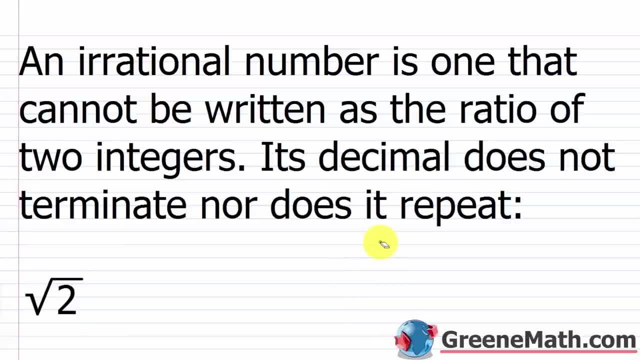 There are no two integers that I can put over each other to give me that irrational number. So its decimal does not terminate. It does not terminate, nor does it repeat. So something like the square root of 2. You cannot find two integers that you can put over 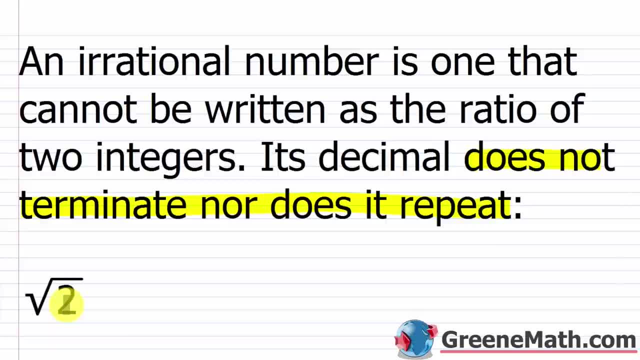 each other that would give you the square root of 2. If you type this into a calculator, you're not going to get an exact value. Your calculator is either going to round, or it's going to truncate. And it's going to give you an estimate for it, but not an exact value. And usually, we'll say this is approximately equal to 1.41. 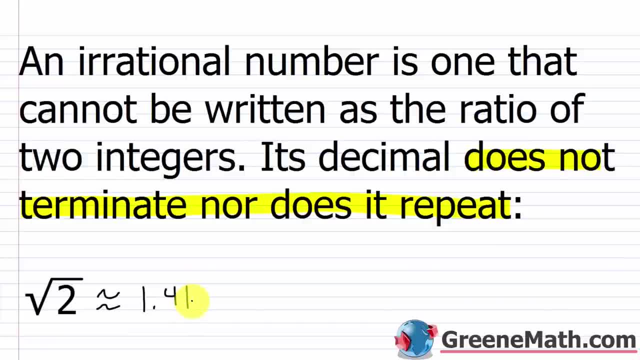 But if you type it up on a calculator, and I just typed it up on mine, I get 1.414213562. So after that final digit that you get, realize that it continues forever and ever and ever. 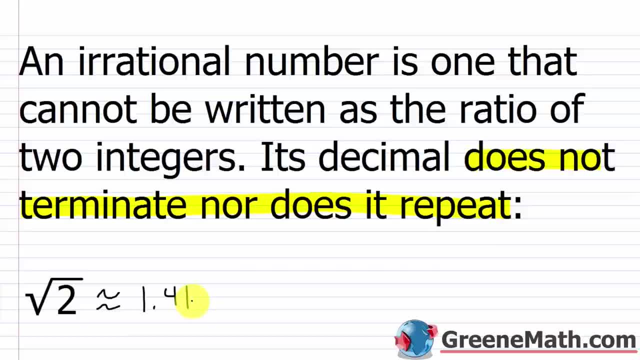 And it's not going to terminate or repeat the same pattern. So that's the problem with an irrational number. You can't really work with it that easily. A famous example of this is pi. 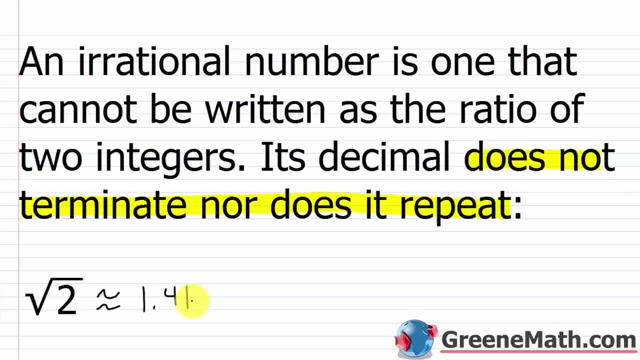 We talked about this before when we talked about direct variation. And I gave you an example where in the Hollywood movie, The Life of Pi, this guy, when he was a child, is on a blackboard, and he's reciting all these digits of pi. And you can go on a computer and go into Google, and you can find websites that give you, all these digits of pi. No matter how many you list, it just keeps going forever and ever. You can't list all of them. So that's the problem, again, with an irrational number. So when we get 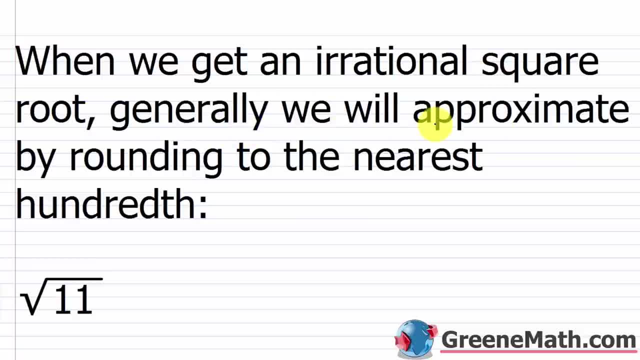 an irrational square root, generally, we will approximate by rounding to the nearest hundredth. 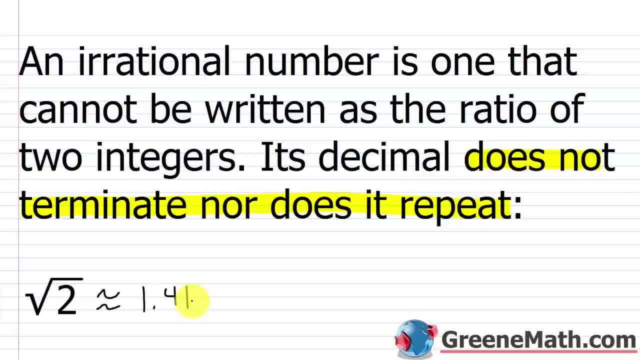 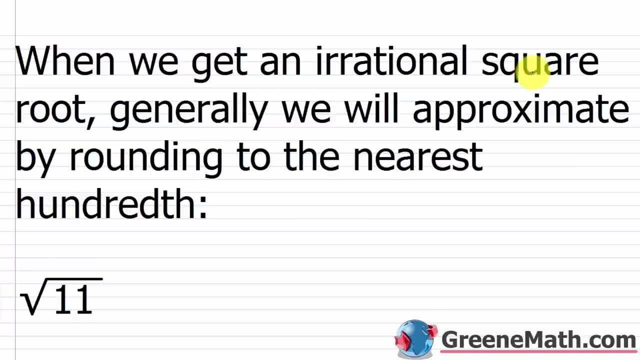 And you can find websites that give you All these digits of pi. No matter how many you list, It just keeps going forever and ever. You can't list all of them, So if we're doing an irrational square root, Generally we will approximate. 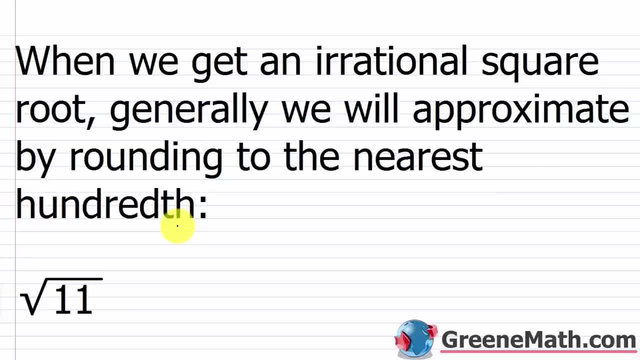 By rounding to the nearest hundredth, And sometimes you won't approximate at all. Sometimes you're just going to leave it like this. But in some cases it's necessary to Kind of do an estimate. In other cases you can kind of leave it like that. 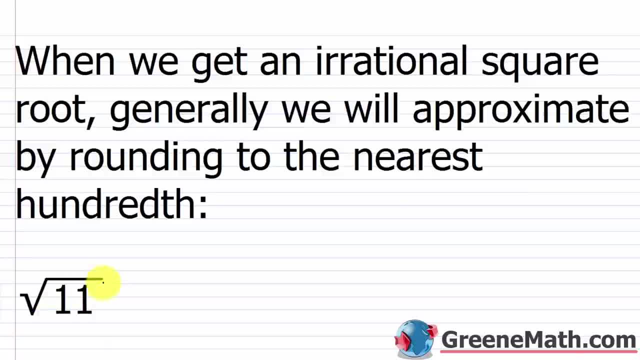 Just depends on the scenario you're dealing with. So square root of eleven, for example, Would be approximately: Punch that up on a calculator To get about three point three, one, You know, six, six, two, four, seven, And let me kind of stop there. 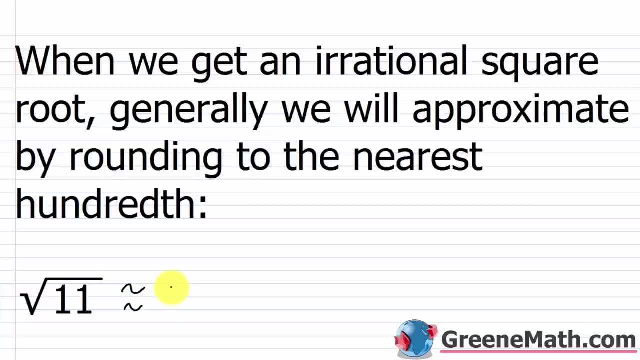 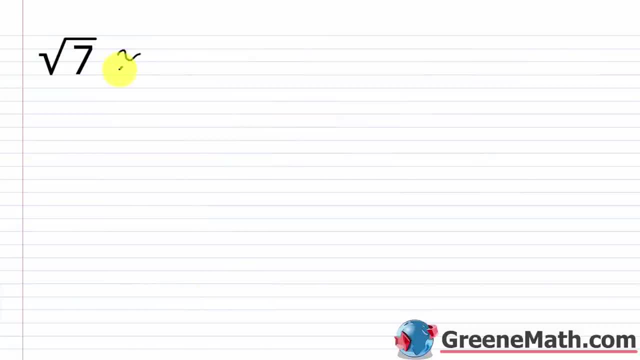 If we ran that to the nearest hundredths That would be three point three, two. So three point three, two. What about square root of seven? So you punch that up on a calculator. If we ran that to the nearest hundredths You'd have something like two point six, five. 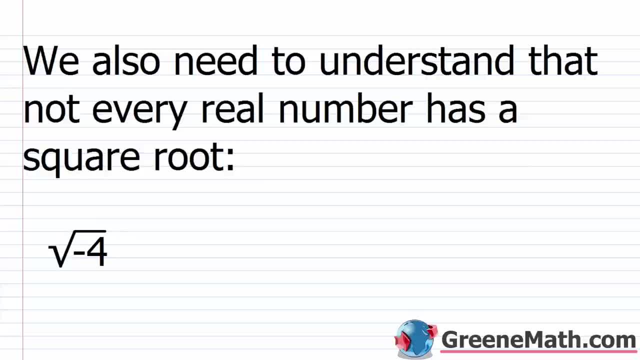 Alright. so now that we understand Kind of the basics of finding the square root of a number And we know the difference in notation Between finding the principal Or positive square root And kind of the negative square root, We've got to move into 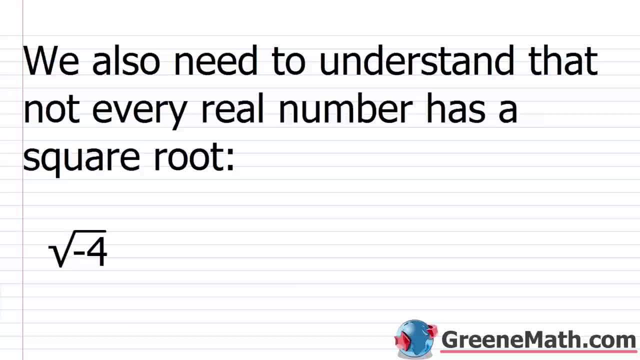 The material. So the first thing that students struggle with Would be the square root Of a negative number. So we also need to understand That not every real number Has a square root. So if I ask you for the square root, 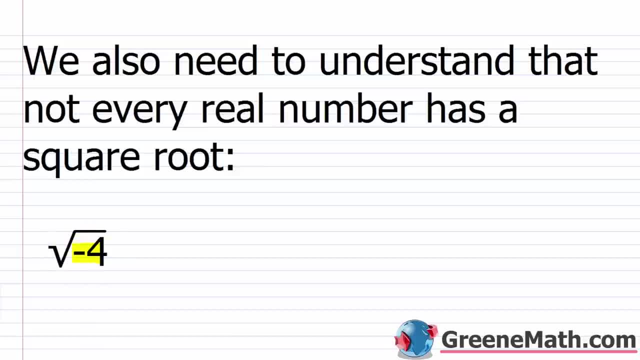 Of negative four. What am I asking you for? The first thing students might do Is they might get confused and say: well, I'm thinking back through this lesson that we just had, And he already covered this- That the square root of four. 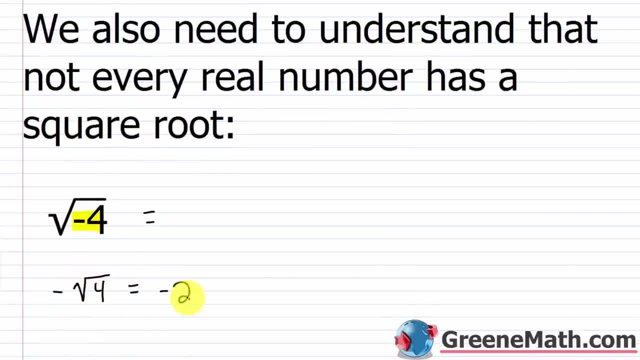 This equals negative two. No, that's not what I'm talking about. In this case, The number under the square root symbol Is a four. It is a positive value. The negative is outside. This is outside. That's a big deal. 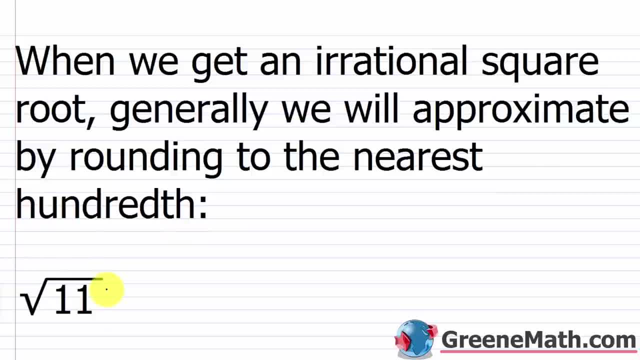 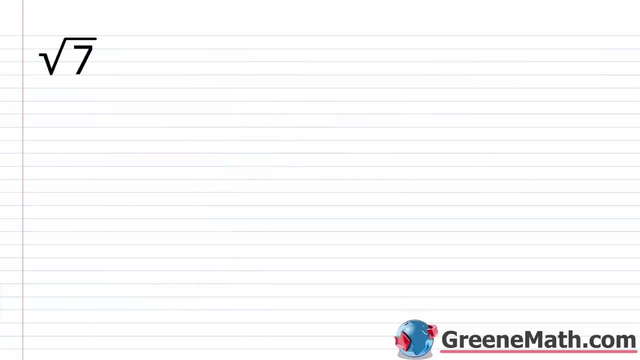 And sometimes you won't approximate at all. Sometimes you're just going to leave it like this. But in some cases, it's necessary to kind of do an estimate. In other cases, you can kind of leave it like that. Just depends on the scenario you're dealing with. So square root of 11, for example, would be approximately. Punch that up on a calculator to get about 3.3166247. And let me kind of stop there. If I ran it to the nearest hundredths, that would be 3.32. So 3.32. What about square root of 7? So you punch that up on a calculator. If we ran it to the nearest hundredths, 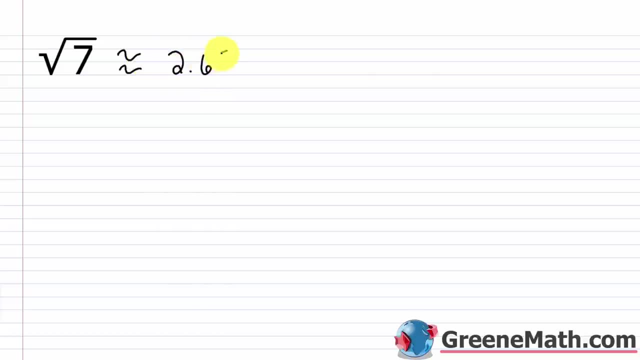 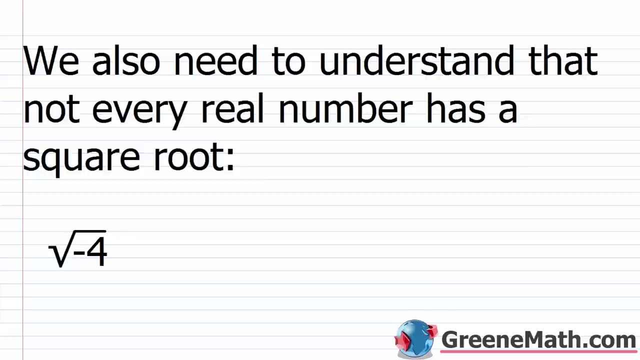 you'd have something like 2.65. All right. So now that we understand kind of the basics of finding the square root of a number, and we're going to go ahead and do a little bit of math, we're going to the difference in notation between finding the principal or positive square root and kind of the negative square root, we've got to move into some kind of harder material. So the first thing that 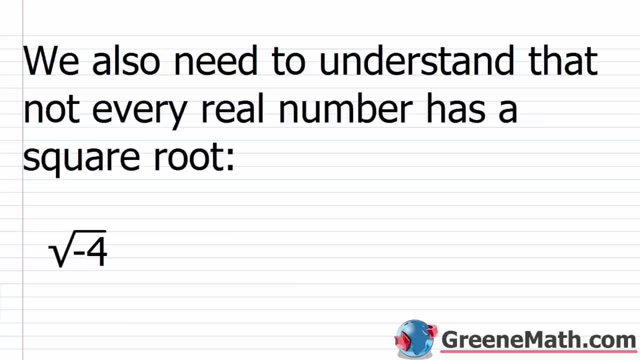 students struggle with would be the square root of a negative number. Okay. So we also need to understand that not every real number has a square root. So if I ask you for the square root of negative four, what am I asking you for? The first thing students might do, is they might get confused and say, well, I'm thinking back through this lesson that we just had, and he already covered this. This is negative square root of four. This equals negative two. 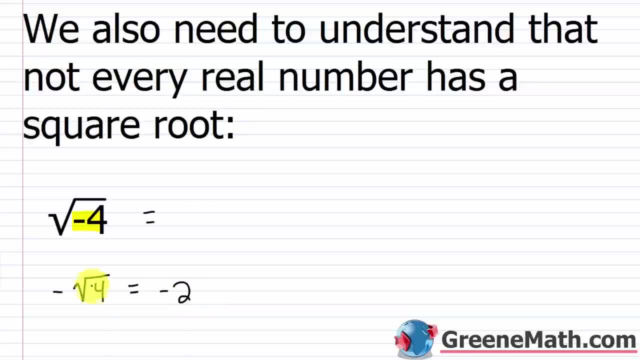 No, that's not what I'm talking about. In this case, the number under the square root symbol is a four. Okay. It is a positive value. The negative is outside. This is outside. Okay. That's a big deal. Now, in this particular case, I have the negative four inside this little symbol. So what I'm saying is what number when multiplied by itself is going to give me negative four? The answer to that is it does not exist. Okay. Now, when we get higher in math, we're thinking about these imaginary numbers, but in our real number system does not exist, right? You can't square a number and get a negative number, right? You can't do that because a negative times another negative is going to give you a positive. 100% of the time. So there's no number that if I multiply by itself is going to give me a negative four. So we would just put not a real number. Okay. It doesn't exist. And you can try that on your calculator. And depending on the calculator, you might get no real answer. You might get not a real number. You might just get error, so on and so forth, because the computer cannot calculate a number that when multiplied by itself is going to give you a negative four. 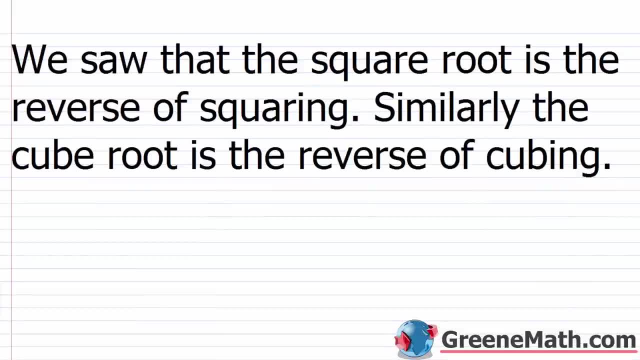 All right. So now let's move on and talk about some higher level roots. So we saw that the square root is the reverse of squaring. So similarly, the cube root is the reverse of cubing. So cubing is nothing more than just raising something to the third power. So in other words, if I had two cubed, this is what this is two times two times two, or just the number eight. So if I reverse that process, and I said, here's my eight here, the symbol looks the same. 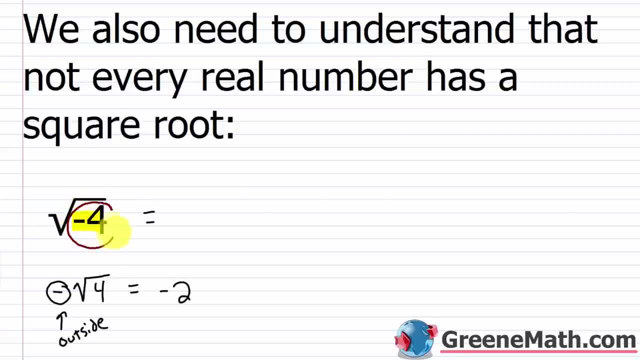 Now, in this particular case, I have the negative four inside This little symbol. So what I'm saying is That every number, When multiplied by itself, Is going to give me negative four. The answer to that is: it does not exist. 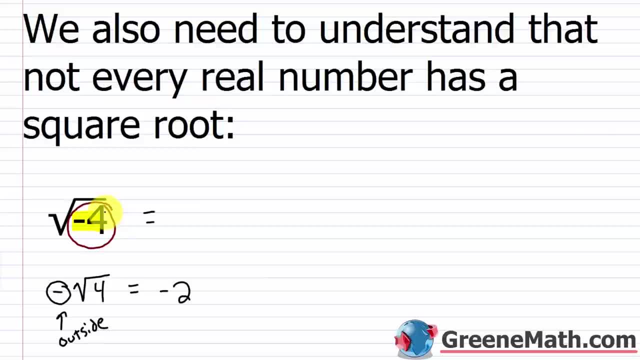 Now, when we get higher in math, We're thinking about these imaginary numbers, But in our real number system Does not exist. You can't square a number And get a negative number. You can't do that Because a negative Times another negative. 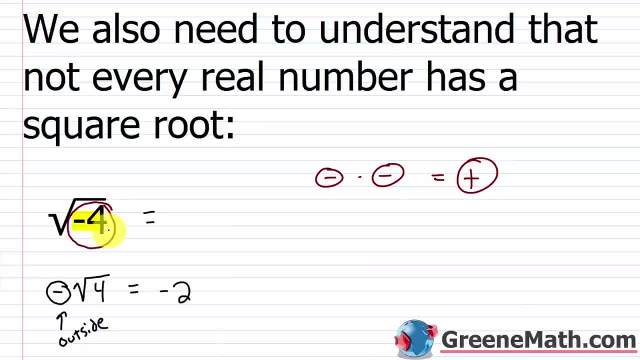 Is going to give you a positive. 100% of the time It's going to give me a negative four. So we would just put Not a real number, It doesn't exist And you can try that on your calculator And, depending on the calculator, 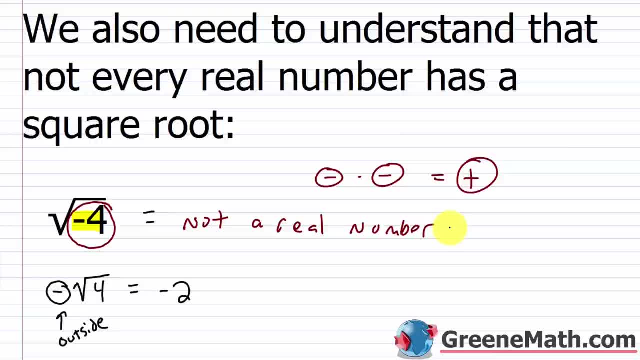 You might get no real answer, You might get not a real number, You might just get error, So on and so forth, Because the computer cannot calculate a number That, when multiplied by itself, Is going to give you a negative four. Alright, so now let's move on. 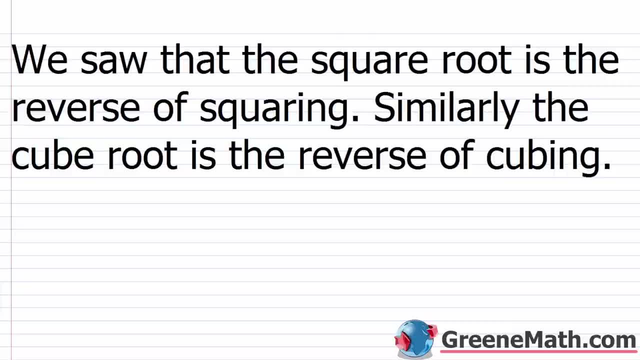 And talk about some higher level roots. The cube root is the reverse of squaring. So, similarly, The cube root is the reverse of cubing. So cubing is nothing more than Just raising something to the third power. So in other words, 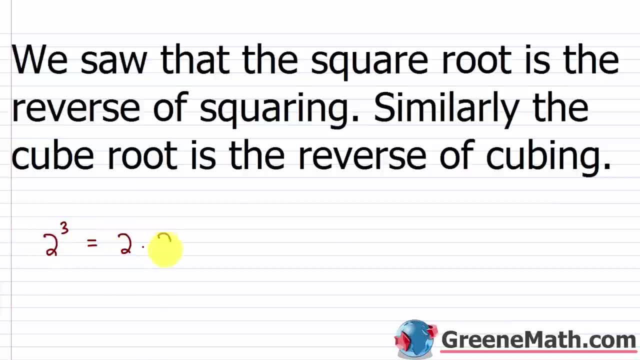 If I had two cubed. This is what This is, two times two times two, Or just the number eight. So if I reverse that process And I said Here's my eight, here The symbol looks the same. All I'm going to do is: 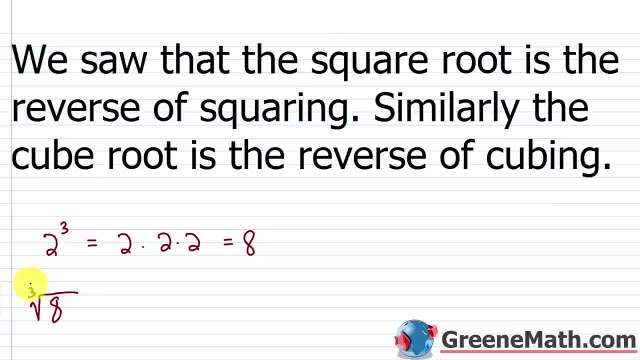 That tells me I want the cube root of eight, Or I want a number That, when multiplied by itself Three times, Is going to give me eight, And we know the answer to that is two. Alright, so in general, When we work with roots, 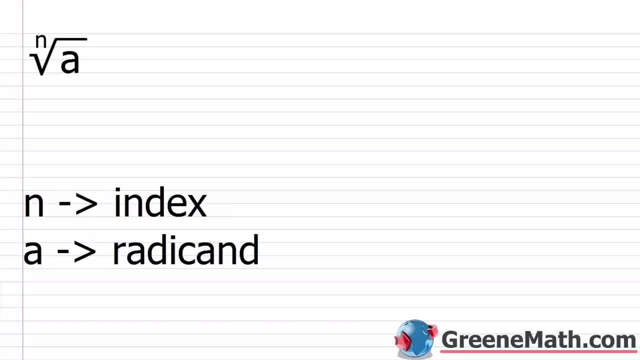 Not just square roots, but roots in general. You kind of think about A. The number that is underneath the symbol Is known as the radicand. So this is the radicand. This is something They might test you when you first get to square roots. 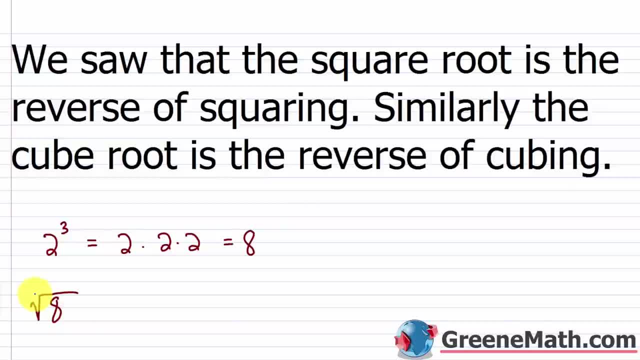 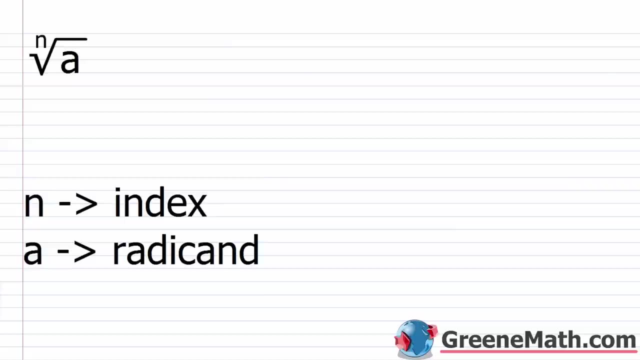 All I'm going to do is instead of having nothing here, I'm going to put a three that tells me I want the cube root of eight, or I want a number that when multiplied by itself three times, okay, three times is going to give me eight. And we know the answer to that is two. All right. So in general, when we work with roots, okay, not just square roots, but roots in general, you kind of think about, okay, a, the number that is underneath the symbol is known as the radicand. So this is the radicand. This is something that they might test you on when you first get the square root. So this is the radicand. And is known as the index. Okay, this is the 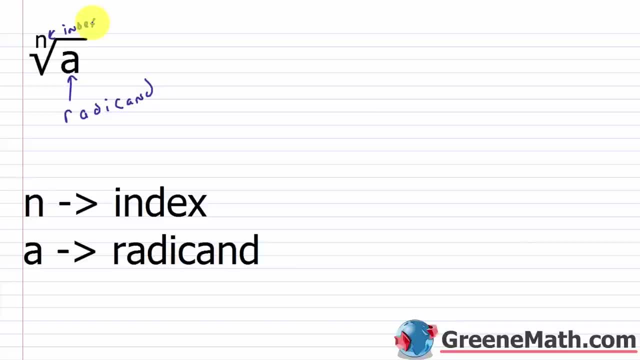 index. And the index is important because it tells me what I'm looking for. So for example, when I just saw the cube root of eight, my index is three, right, my radicand is eight. 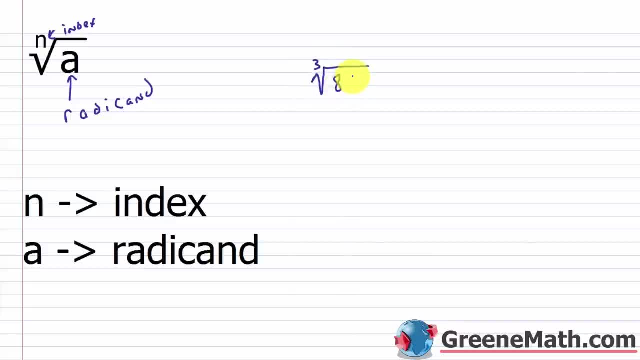 So I'm saying what number, again, when multiplied by itself three, times would give me eight. If I had something like, let's say the fourth root of 16, okay, I'm doing easy stuff. The fourth root of 16 is asking what number when multiplied by itself four times is going to give me 16. Well, we would think about two. You could also have negative two, right, but it would be a different notation. But two times two is four times two again is eight times two one more time is 16. And again, you could also, say the fourth root of 16 would be negative two. But again, there's that different notation for that. Now, this symbol here is known as just a radical symbol, a radical symbol. 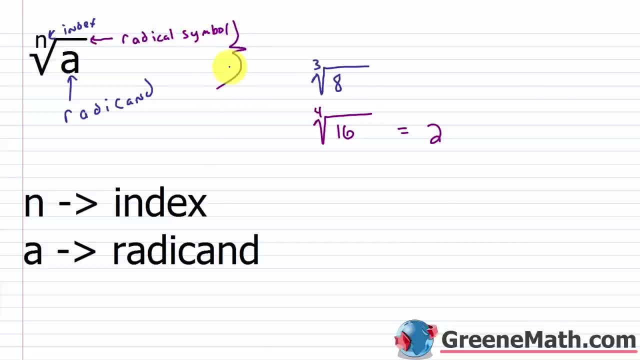 And then the whole thing, okay, so the whole thing is known as a radical. 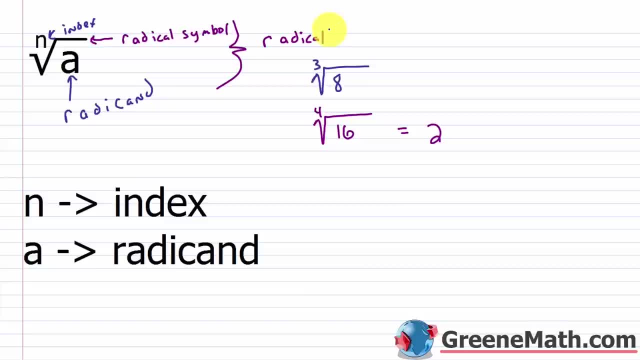 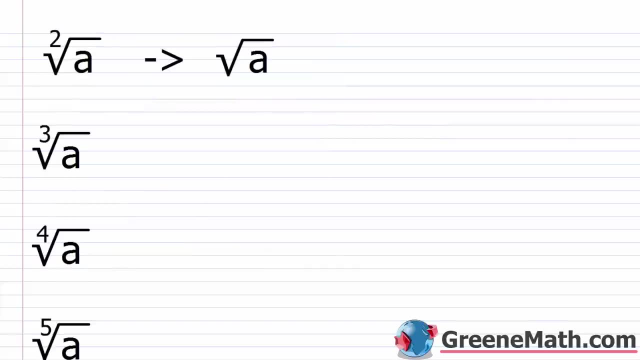 So if your teacher comes in and says, we're studying radicals today, or we're studying numbers today, okay, they're basically talking about the same thing. Now, one thing you would have noticed already is that when we have the square root, we don't write the two, right? The index would be a two, but we don't write it, it's left blank. So that's one property of square roots. 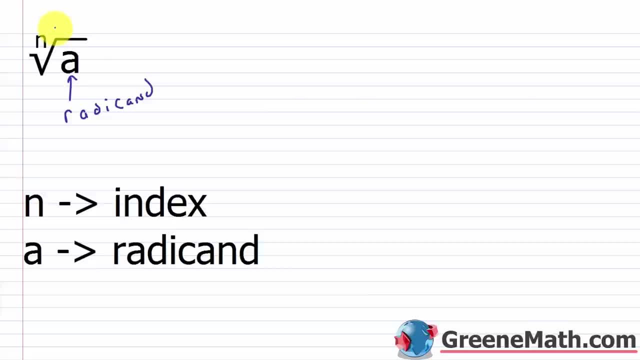 So this is the radicand. N is known as the index. This is the index, And the index is important Because it tells me What I'm looking for. So, for example, When I just saw the cube root of eight, 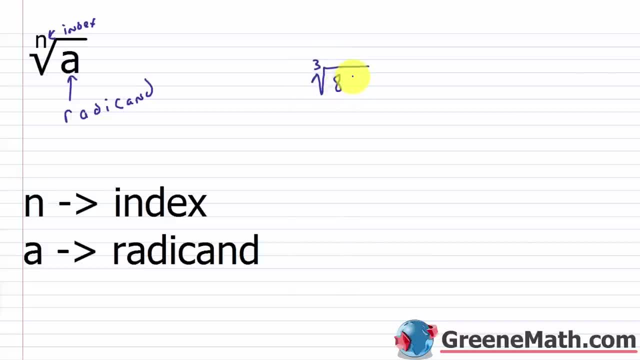 My index is three, My radicand is eight. So I'm saying: what number Again, when multiplied by itself, three times Would give me eight, If I had something like The fourth root of sixteen. Okay, I'm doing easy stuff. 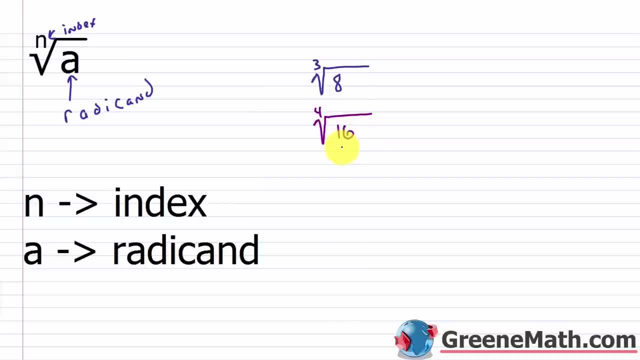 The fourth root of sixteen is asking What number, when multiplied by itself four times, Is going to give me sixteen. Well, We would think about two. You could also have negative two, But it would be a different notation. But two times two is four. 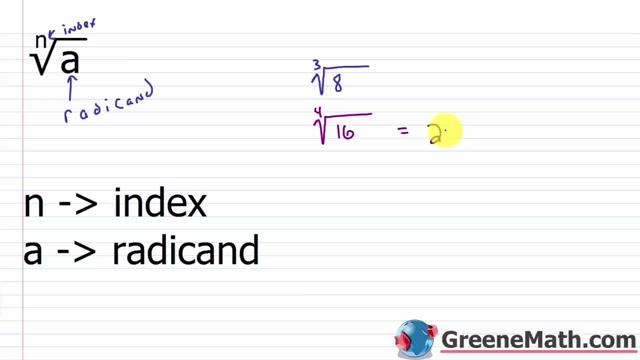 Times two. again is eight, Times two. one more time is sixteen. And again you could also Say the fourth root of sixteen would be negative two, But again there's that different notation for that. Now this symbol here Is known as Just a radical symbol. 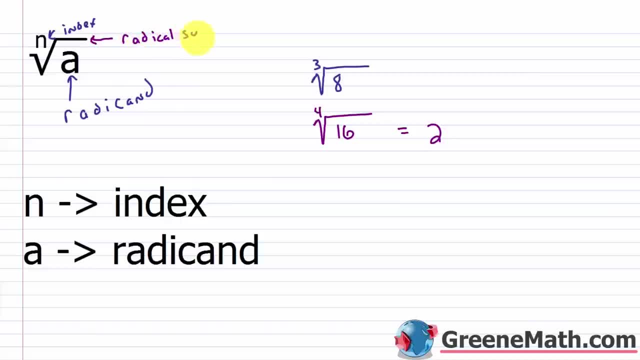 A radical Symbol, And then the whole thing: Okay. so the whole thing Is known as a radical. So if your teacher comes in and says We're studying radicals today Or we're studying roots today, Okay, They're basically talking about the same thing. 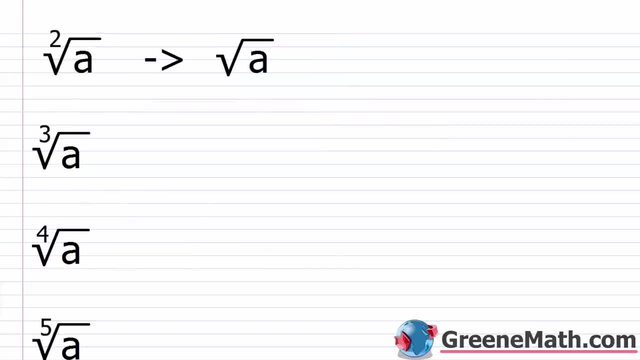 Now one thing you would have noticed already: When we have the square root, We don't write the two. The index would be a two, But we don't write it. It's left blank. So that's one property of square roots. 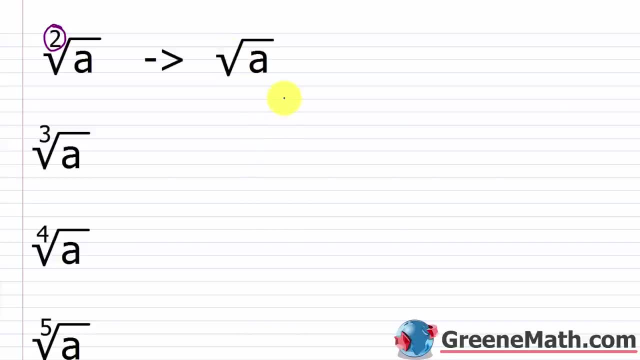 If you write a two up there, It's not incorrect, It's just not traditional. So if I put the square root of, Let's say, sixteen like that, It's the same thing as if I put the square root of sixteen like that. 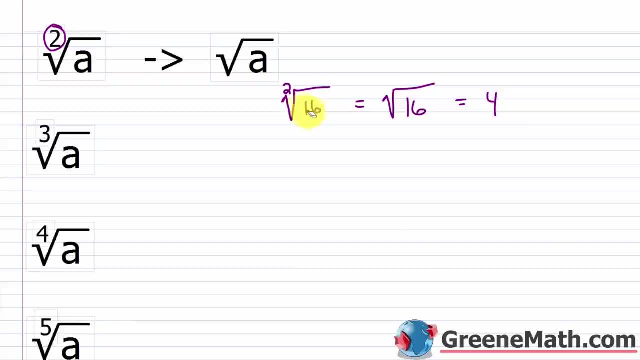 In each case it's four. This is just a notational thing that we do, So this one right here. If I have an index of three, This is the cube root. If I have an index of four, It's the fourth root. 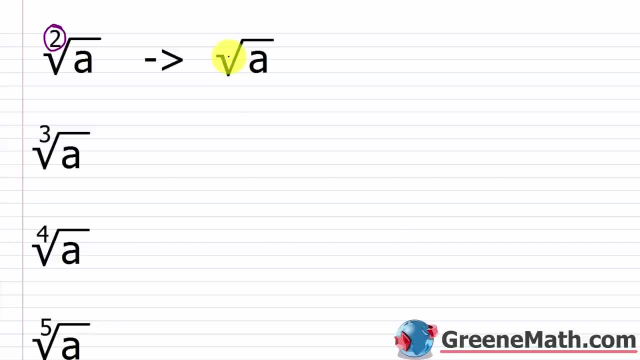 If you write a two up there, it's not incorrect. It's just not traditional. So if I put, you know, the square root of let's say 16, like that, it's the same thing as if I put the square root of 16, like that, right? In each case, it's four. This is just a notational thing that we do. So this one right here, if I have an index of three, 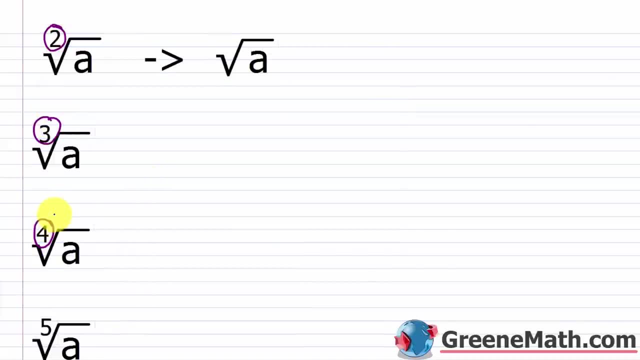 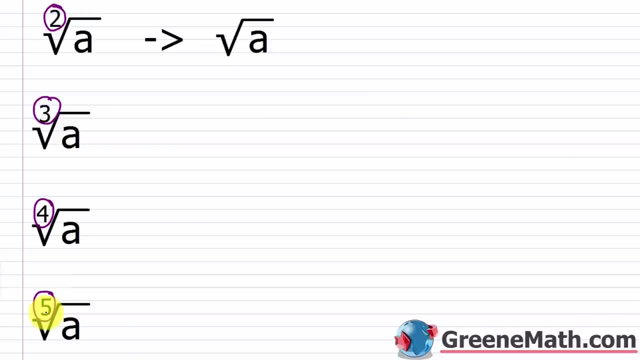 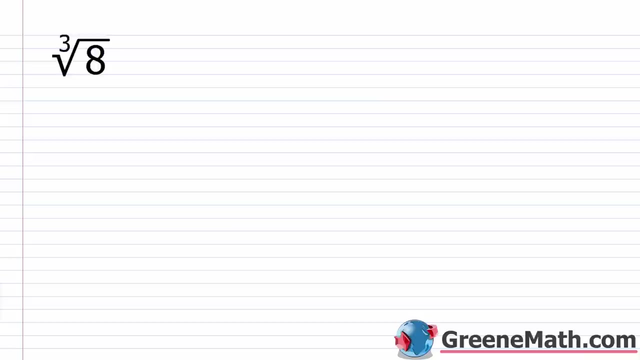 this is the cube root. If I have an index of four, it's the fourth root. If I have an index of five, it's the fifth root, right? So on and so forth. You can put any number you want there, but it starts getting very, very complex. If I'm looking for the fifth root of something, I'm looking for a number that when multiplied by itself five times gives me that number, the radicand. So again, let's look at some easy examples of this. If I have the cube root of eight, again, what number when multiplied by itself three times gives me eight, we know at this point that that's two, right? Two times two is four, four times two is eight. So now we have the fourth 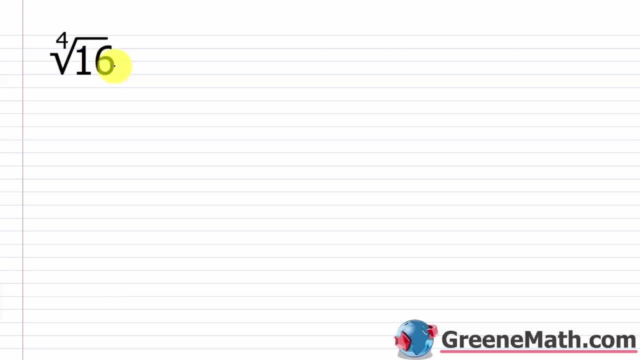 root of 16, which we already looked at. Again, what number when multiplied by itself four times gives me 16? Well, that's going to be two. And this is the principal fourth root of 16. So I want a negative two. If I want a negative two, then I would look at the negative fourth root of 16. In this case, this is negative two. This one is one you have to pay attention to. We know that in the case of a square root, so let's say I want the square root of negative 16. I already talked about 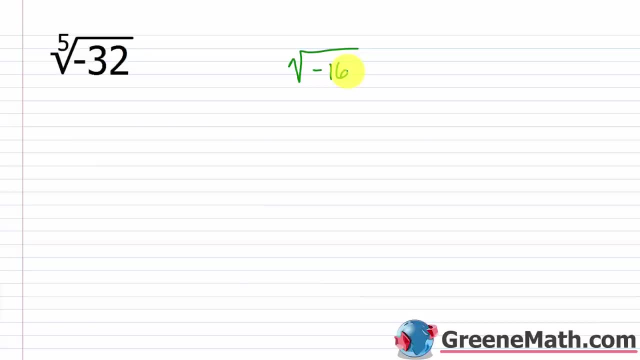 the fact that that's not a real number, right? I can't square a number and get a negative result. Negative times negative is positive. Negative times negative is positive. Negative times negative is positive. If I'm asking for an even root, so something to the second power, let's say to the fourth power, you know, so on and so forth, this is not going to be a real number, right? It's not going to be possible, right? Because an even number of negative signs when multiplied together gives you a positive. If I have an odd index, like I have here, it is possible, right? Because an odd 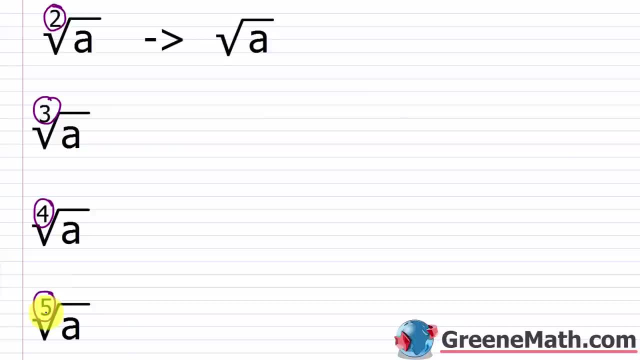 If I have an index of five, It's the fifth root, So on and so forth. You can put any number you want there, But it starts getting very, very complex. If I'm looking for the fifth root of something, I'm looking for a number. 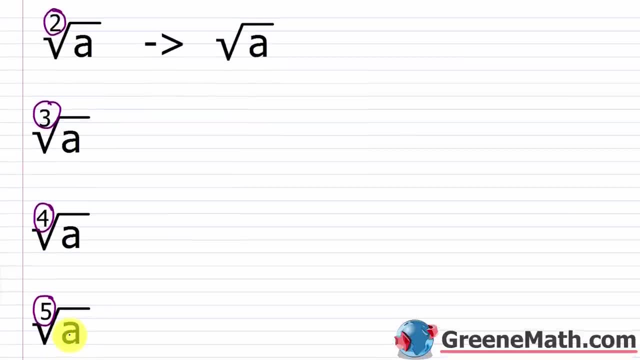 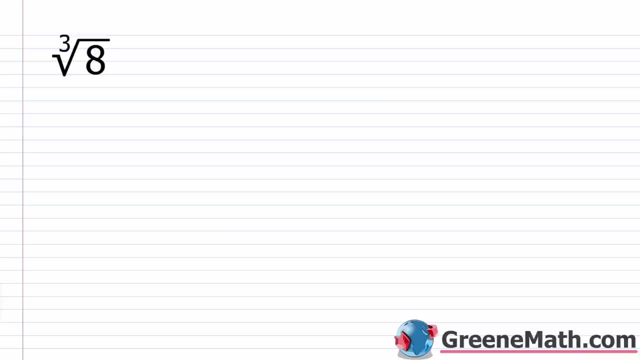 That, when multiplied by itself five times, Gives me that number. And let's look at some easy examples of this. If I have the cube root of eight, Again what number, When multiplied by itself three times, Gives me eight? We know at this point that that's two. 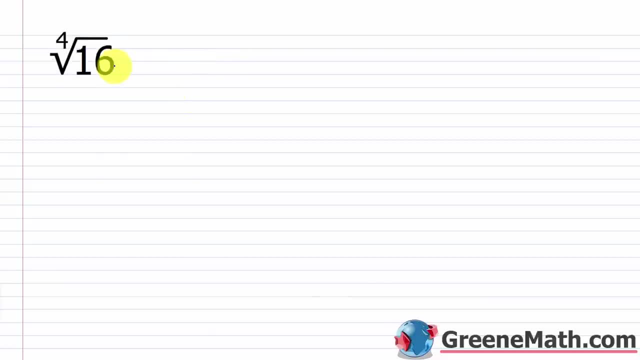 Two times two is four. Four times two is eight. So now we have the fourth root of sixteen, Which we already looked at Again. what number, When multiplied by itself, four times, Gives me sixteen? Well, that's going to be two. 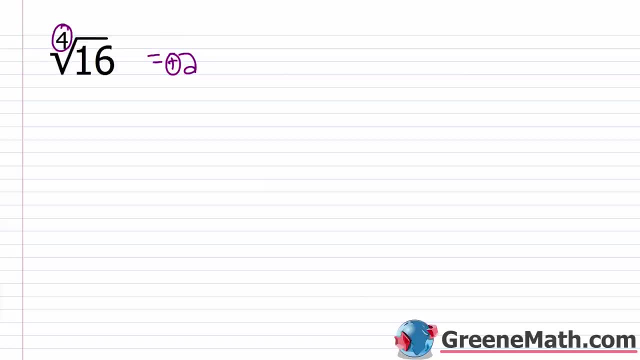 And this is the principle. If I want a negative two, Then I would look at the negative Fourth root of sixteen. In this case, this is negative two. This one is one you have to pay attention to. We know That in the case of 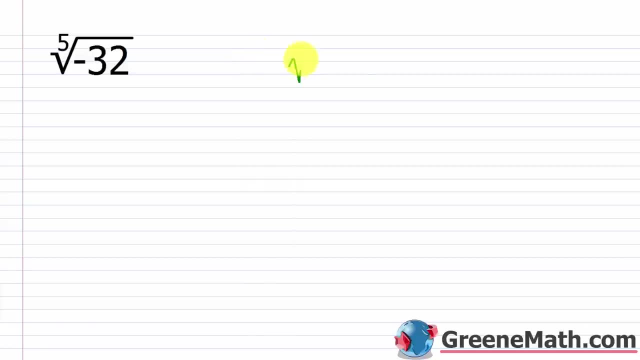 A square root. So let's say I want the square root Of negative sixteen. I already talked about the fact That that's not a real number. I can't square a number And get a negative result. Negative times: negative is positive. 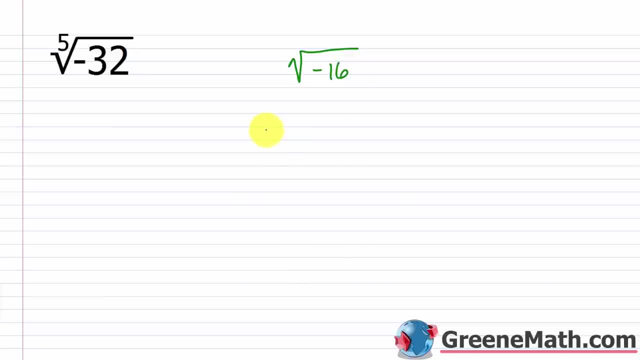 If I'm asking for An even root, So something to the second power, Let's say to the fourth power, You know, so on and so forth. This is not going to be A real number, It's not going to be possible. 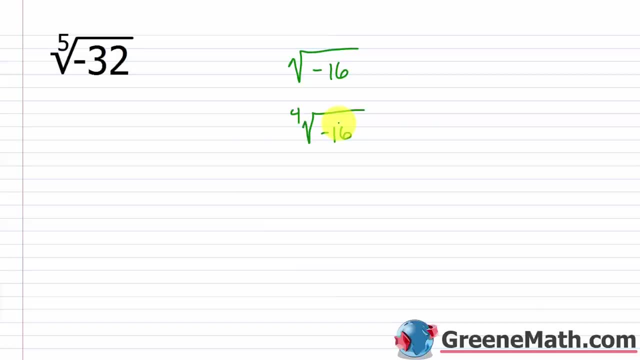 Because an even number of negative signs, When multiplied together, Gives you a positive. If I have an odd index, like I have here, It is possible Because an odd number of negative signs Can in fact give me a negative result. So if I had something like 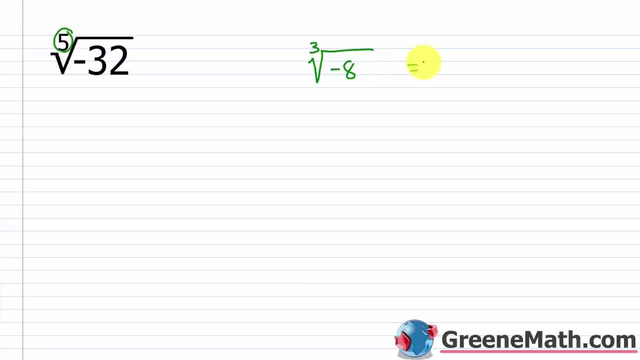 The cube root of negative eight. This is a real number. It's negative two, Negative two times negative. two is positive four. Positive four times negative. two is negative eight. In this case we have five. Five is an odd number, So I can have the fifth root of negative thirty two. 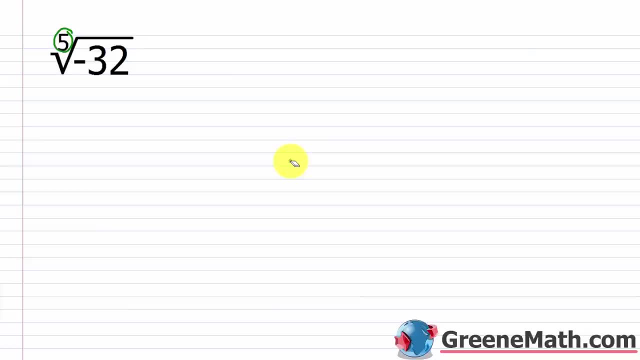 number of negative signs would, in fact, give me a negative result. So if I had something like the cube root of negative eight, this is a real number. It's negative two. Negative two times negative two is positive four. Positive four times negative two is negative eight. In this case, we have five. Five is an odd number. So I can have 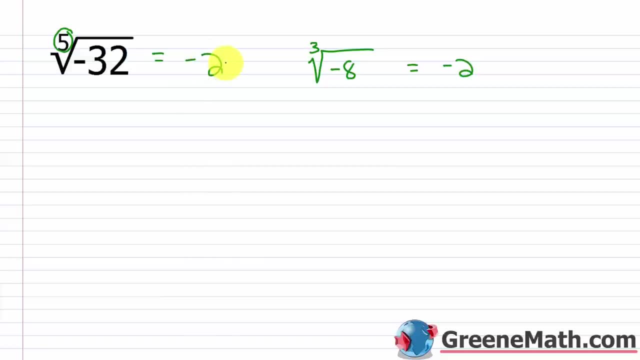 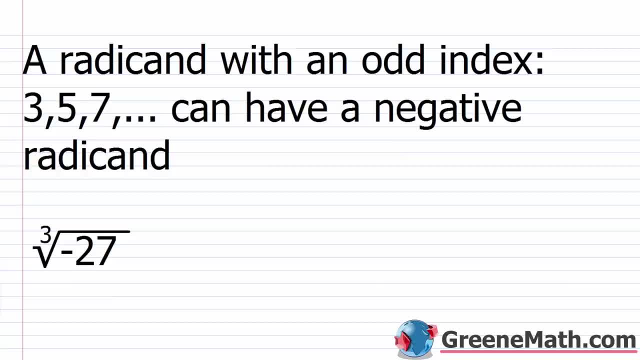 again, the fifth root of negative 32 would be negative two. So again, a radicand with an odd index, three, five, seven, nine, 11, you know, so on and so forth, can have a negative radicand. 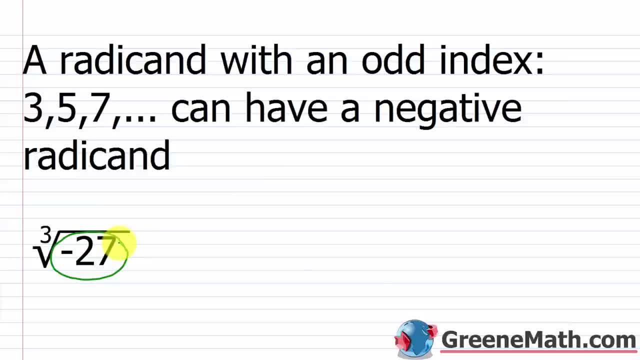 So this part right here can be negative. Again, you have an odd index. If you have an even index, it cannot be. And the reason for that, 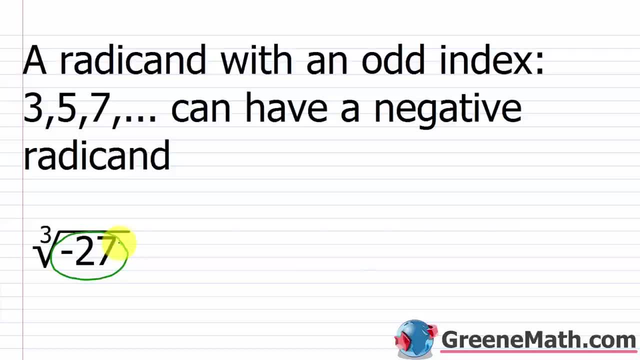 again, is you won't have a real number that will satisfy that. So if I look at the cube root of negative 27, what number, when multiplied by itself three times, would give me negative 27? 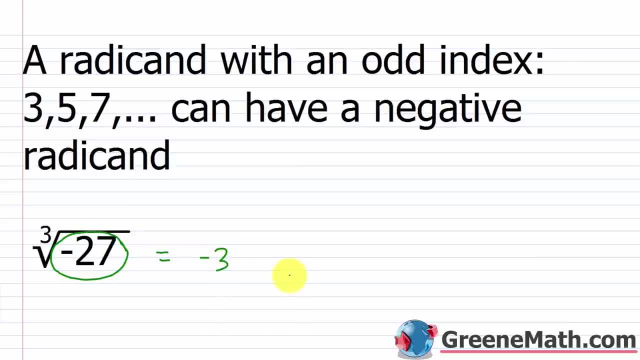 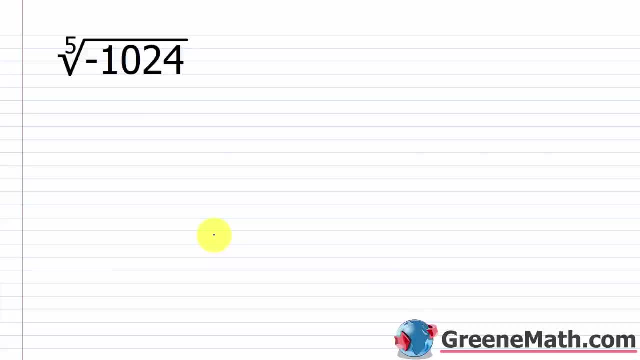 Will it be negative three? Negative three times negative three is positive nine. Positive nine times negative three is negative 27. So let's look at the fifth root of negative 1024. So again, 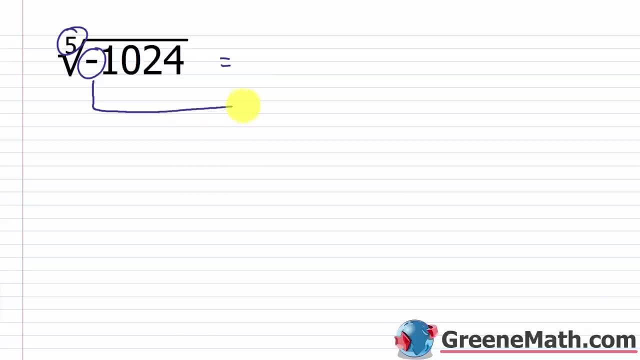 if I have an odd index, this can be negative. And when I'm solving a problem like this, I would just automatically write a negative there, right? If I had five negatives, I would get a negative. So I 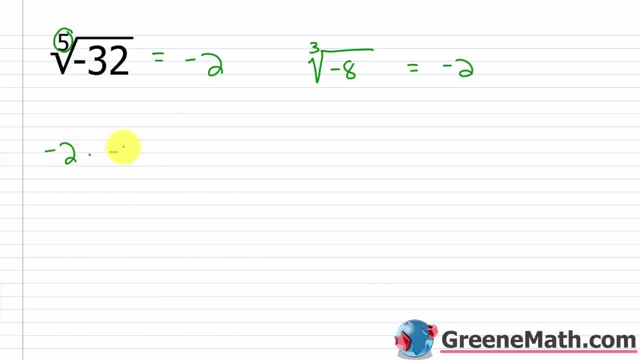 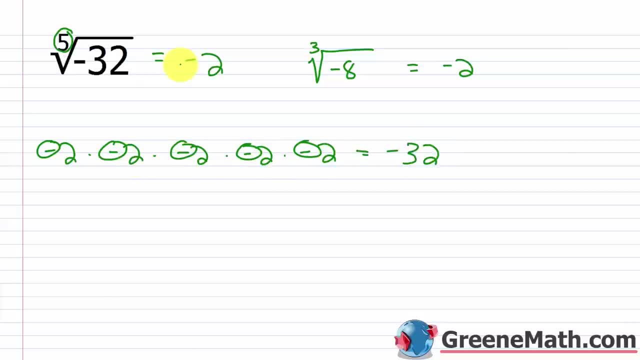 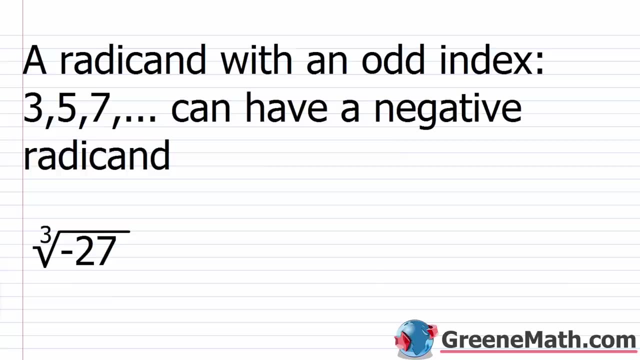 Times two is eight. Times two is sixteen. Times two is thirty two. So that is negative thirty two. And so again the fifth root of negative thirty two Would be negative two. So again a radicand with an odd index. Three, five, seven, nine eleven. 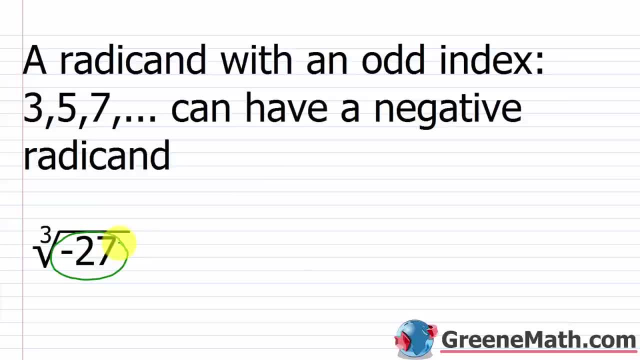 You know, so on and so forth Can have a negative radicand. So this part right here can be negative Again. If you have an odd index, It cannot be, And the reason for that again is You won't have a real number. 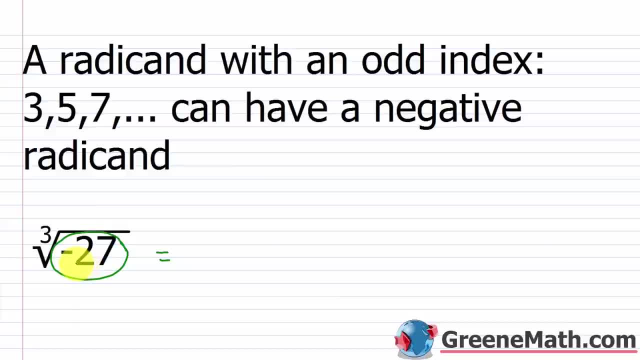 That will satisfy that. So if I look at the cube root of negative twenty seven, What number, When multiplied by itself three times, Would give me negative twenty seven? Will it be negative three? Negative three times negative? three is positive nine. Positive nine times negative three is negative twenty seven. 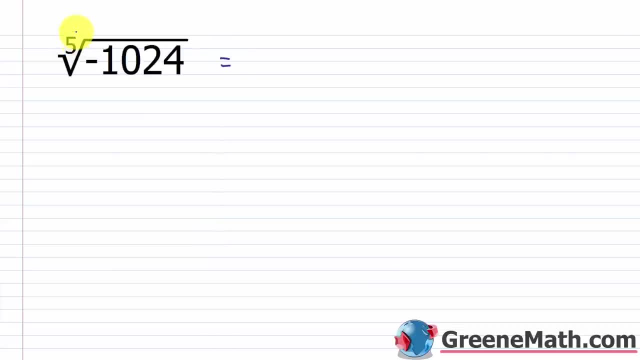 So let's look at the fifth root of negative one thousand twenty four. So again, if I have an odd index, This can be negative, And when I'm solving a problem like this, I would just automatically write a negative there, Right? If I had five negatives. 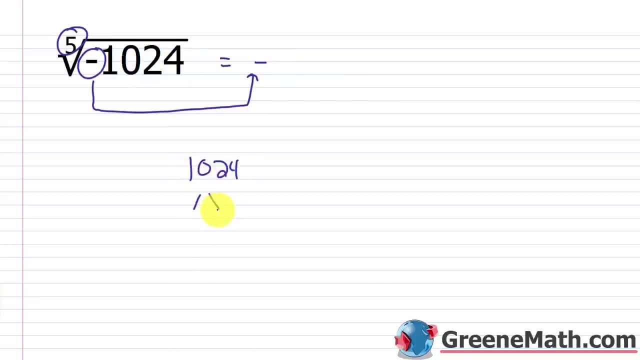 I would get a negative. So I can just think about the number part. So one thousand twenty four, Kind of break this down with a factor tree. I know it's divisible by four, Because twenty four is If I divide one thousand twenty four by four. 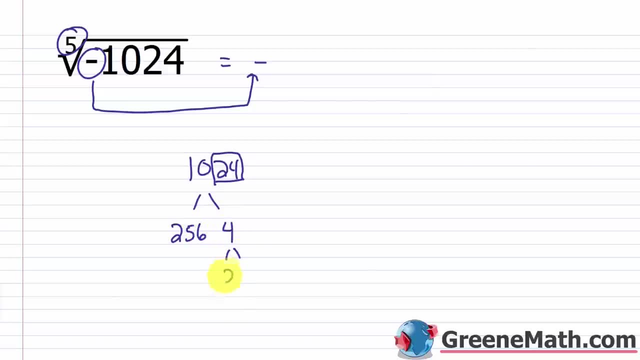 I'd get two hundred fifty six. So two hundred fifty six times four, And four, I know, is two times two. I'm going to double those. So what about two hundred fifty six? Well, I know that's divisible by four. This is four times sixty four. 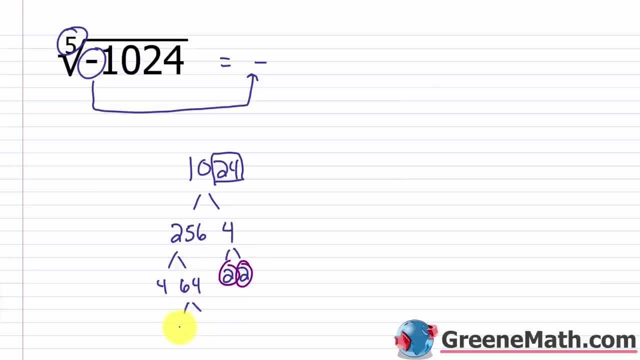 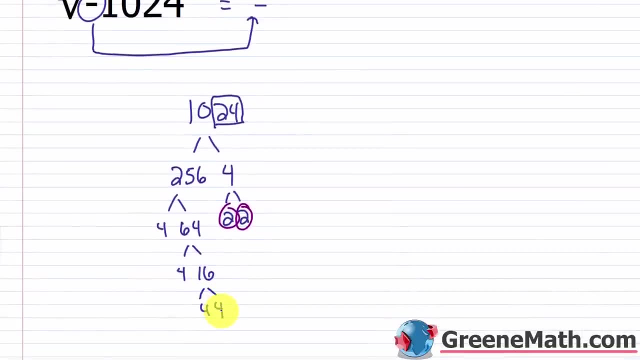 And sixty four is divisible by four, This is four times sixteen. And sixteen is divisible by four, This is four times four. So, without continuing on this factor tree, I've got one, two, three, four And this original one up here: Five factors of four. 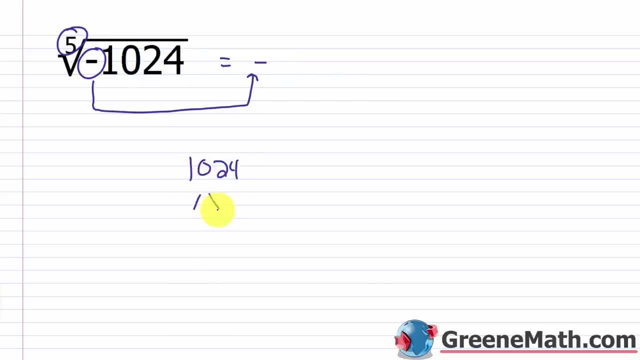 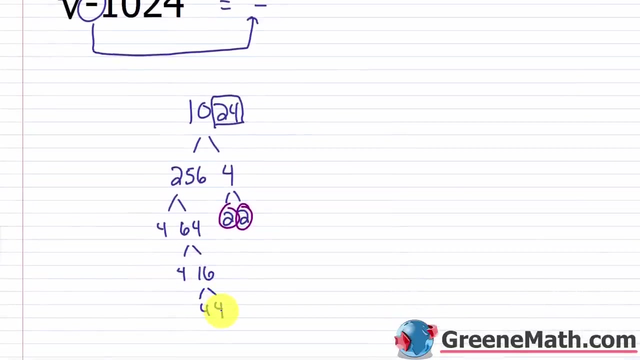 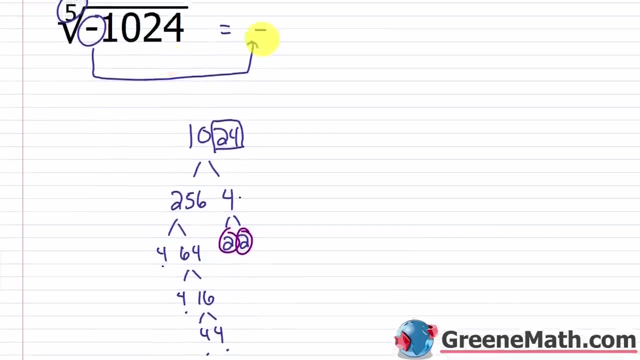 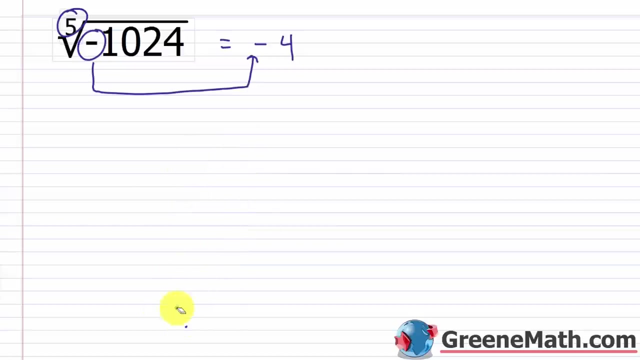 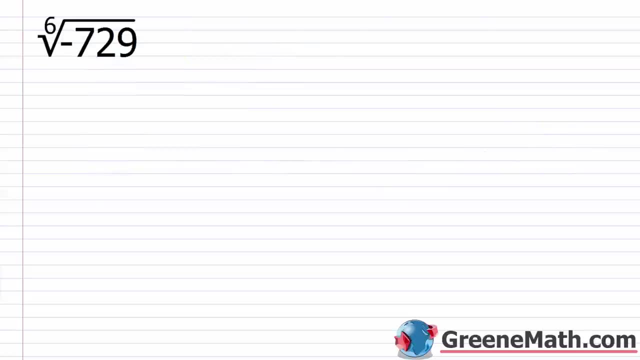 which was my radicand. So then what about the sixth root of negative 729? Do we need to look to solve this? No, because I have a negative here, and I have an even index. So this is not negative. A real number. 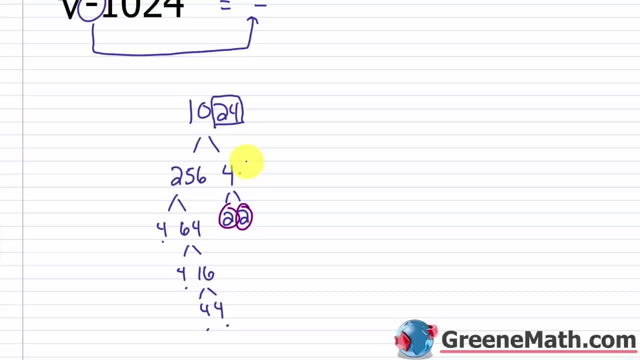 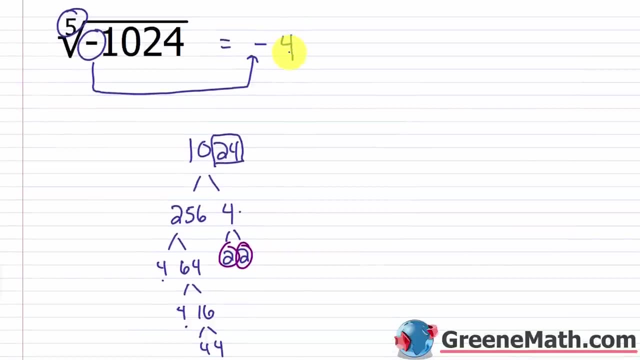 So if I multiplied four times, itself five times, I would get one thousand twenty four, And that's what we're looking for. So this would be negative four As your answer. So let me erase this real quick And I can show that to you real quick. 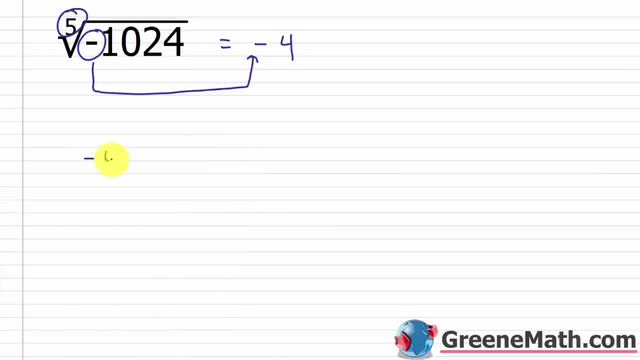 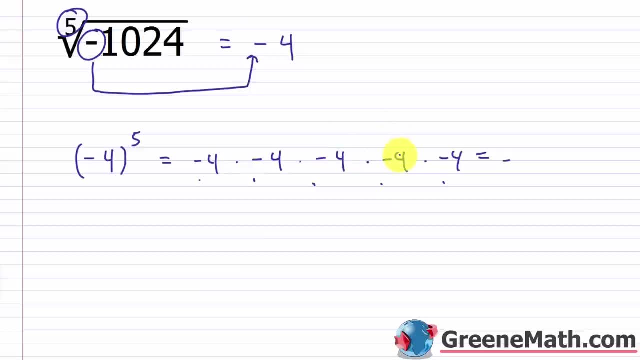 Four times four is sixteen. Negative four is sixty four. Sixty four times four is two hundred fifty six. And if I multiply two hundred fifty six times four, I get a thousand twenty four Right. Stick that next to the negative And I get my negative one thousand twenty four back. 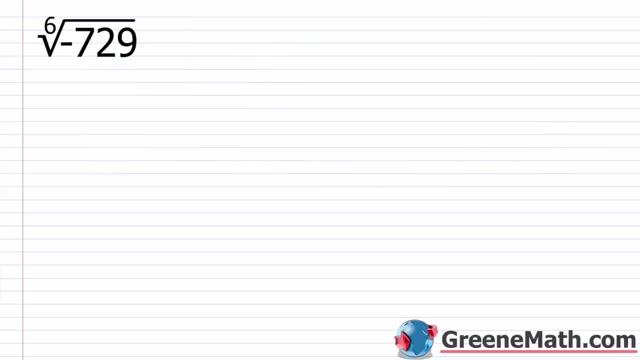 Which was my radicand. So then, what about the sixth root of negative seven hundred twenty nine? Do we need to look to solve this? No, Because I have a negative here And I have an even index, So this is not a real number. 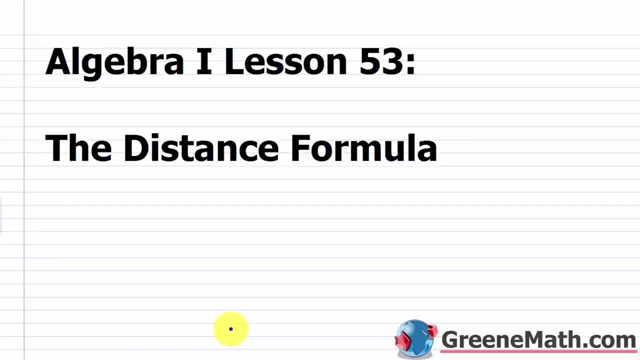 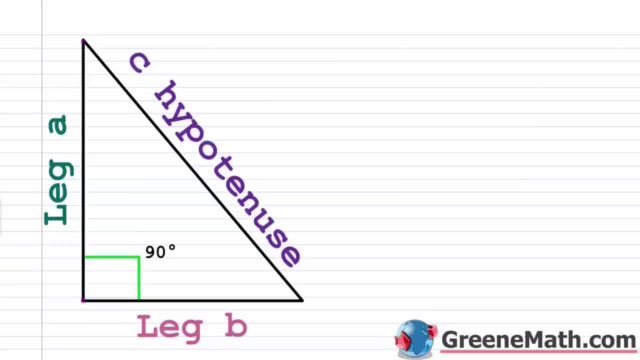 It's just a formula. Hello and welcome to Algebra 1, Lesson 53.. In this lesson we're going to learn about the distance formula. So we just got done talking about square roots, Cube roots, Fourth roots, Basically radicals in general. 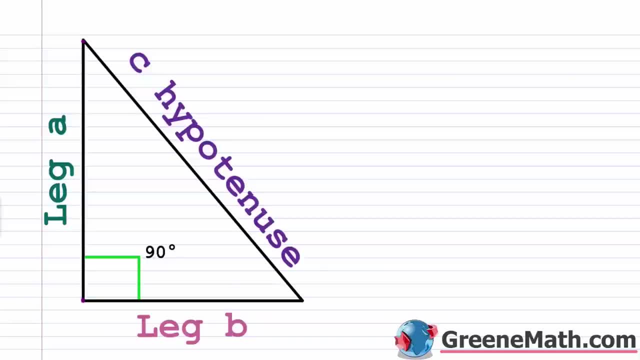 Now, one of the immediate applications of square roots Would be the ability to find the distance Between two points on the coordinate plane Using the Pythagorean theorem, Or your book might say the Pythagorean formula, So the Pythagorean formula. 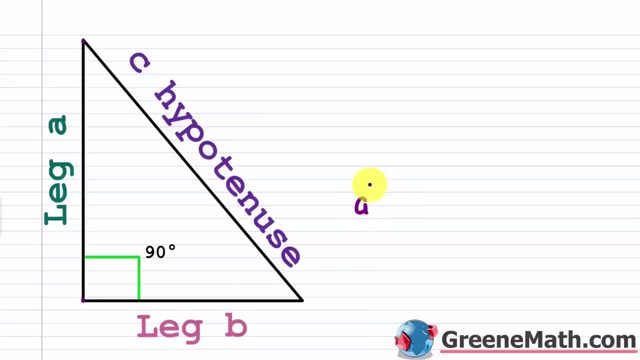 Basically looks like this: You have this: a squared Plus b squared, Equals c squared. It's a pretty famous formula, So even if you haven't taken geometry yet Or you haven't seen it in a previous algebra course, You've probably come across this at some point. 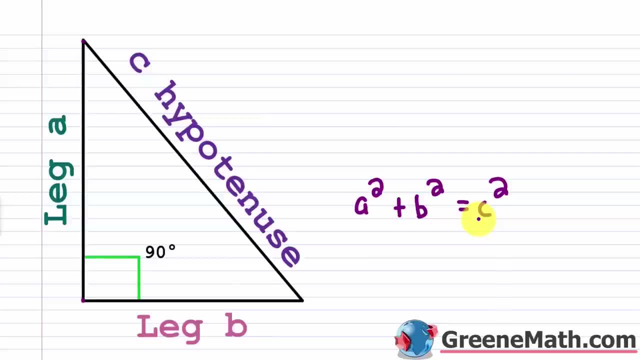 Okay, So what the Pythagorean formula does Is it tells us about the relationship Between the sides in a right triangle. So I alluded to geometry, And I know that some of you probably Haven't studied geometry yet, Because this is usually taken directly. 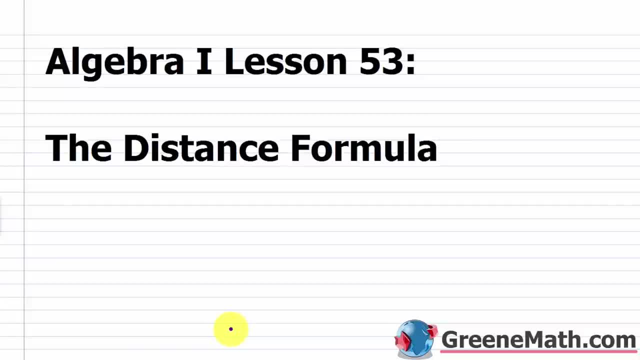 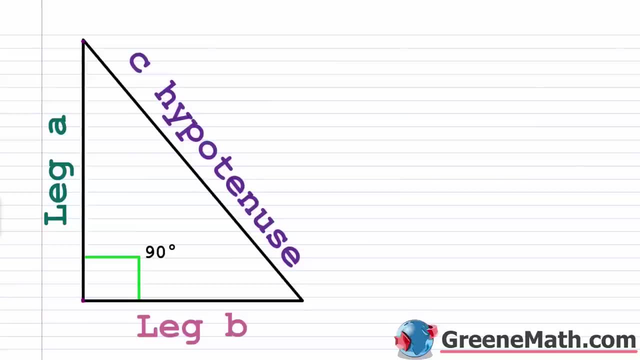 Hello, and welcome to Algebra 1, Lesson 53. In this lesson, we're going to learn about the distance formula. So we just got done talking about square roots, cube roots, fourth roots, basically radicals in general. Now, one of the immediate applications of square roots would be the ability to find the distance between two points on the coordinate plane using the Pythagorean theorem, or your book might say the Pythagorean theorem. So we're going to learn about the Pythagorean formula. So the Pythagorean formula basically looks like this. You have this a squared plus b squared equals c squared. It's a pretty famous formula. So even if you haven't taken geometry yet, or you haven't seen it in a previous algebra course, you've probably come across this at some point, okay? So what the Pythagorean formula does is it tells us about the relationship between the sides in a right triangle. So I alluded to geometry, and I know that some of you probably have heard of it. But I know that some of you probably have heard of it. 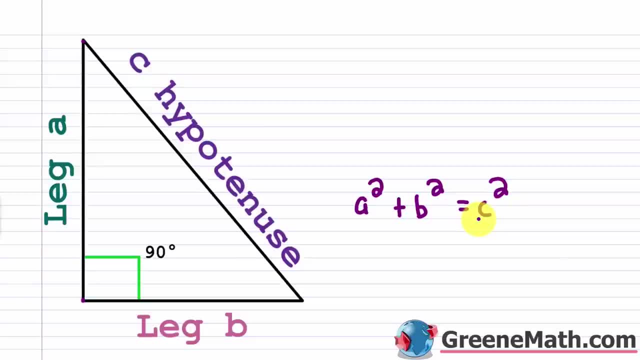 I know that some of you probably haven't studied geometry yet, because this is usually taken directly after an algebra one course. So if you don't know anything about triangles, it's not a big deal. You can pick up what you need to know about right triangles from our lesson today. 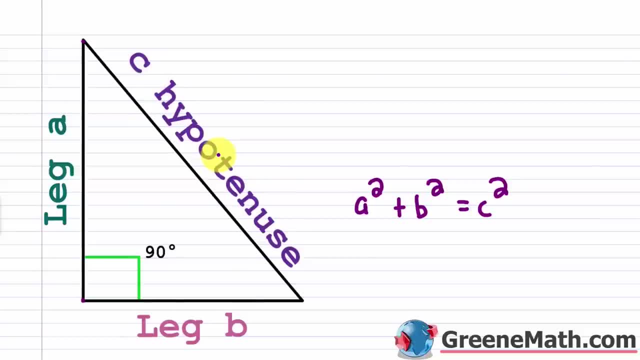 So let's focus on what we have here, this triangle, see a lot of stuff that's labeled, and let's just kind of go through that. So the first thing is you'll notice that this symbol here is going to denote that we have a 90 degree angle, or what is known as a right angle, okay? 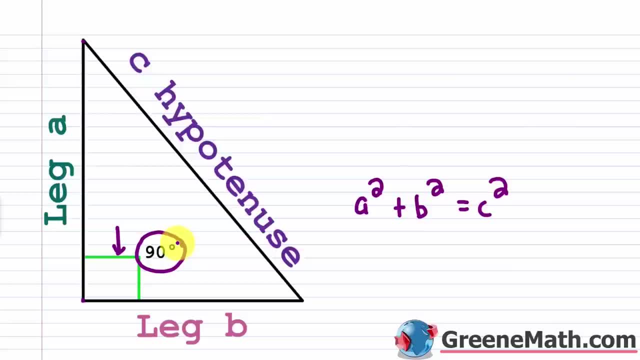 So this triangle has a 90 degree angle, or a right angle. It is known as a right triangle, okay? A right triangle. Now, with a right triangle, you have two shorter sides that are known as legs. So here you have this leg A and this leg B, okay? So those are the two shorter sides of the right triangle. Then the longest side is always going to be opposite of the 90 degree angle. 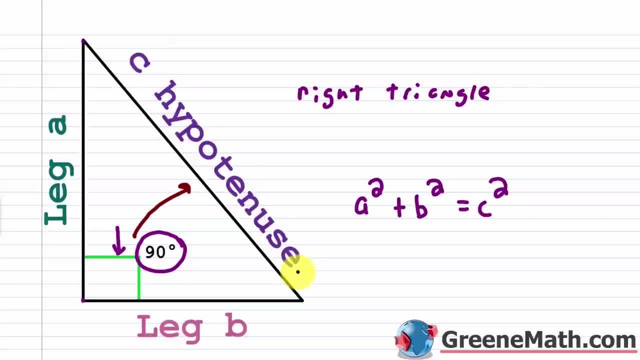 So opposite of that would be here. That's labeled as C, and it's known as the hypotenuse, okay? So the way the Pythagorean formula works is it tells us that kind of the measure of leg A, so from here to here, if we square that, so that's where you get the A squared, then plus the measure of leg B. So from here to here, so you take that and you square it. So you're summing those two amounts together. So A squared plus B squared, this is equal to C, or the hypotenuse, squared, okay? So this is true for any right triangle that you work with. 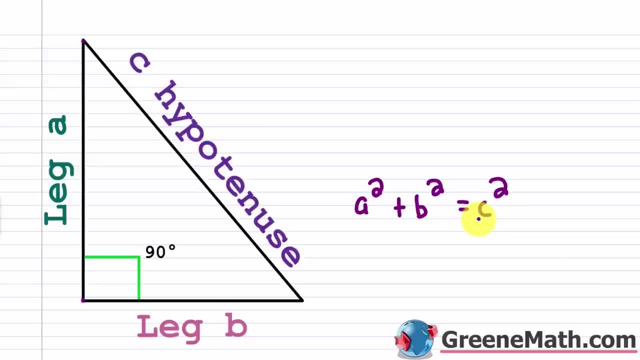 After an algebra 1 course. So if you don't know anything about triangles, It's not a big deal. You can pick up what you need to know about right triangles From our lesson today. So let's focus on what we have here. 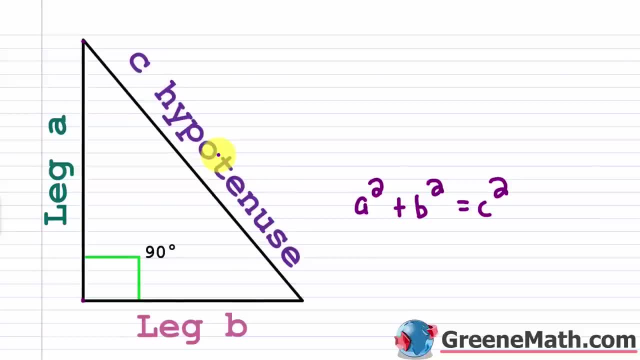 This triangle, See a lot of stuff that's labeled And let's just kind of go through that. So the first thing is, you'll notice that this symbol here Is going to denote that we have a 90 degree angle, Or what is known as a right angle. 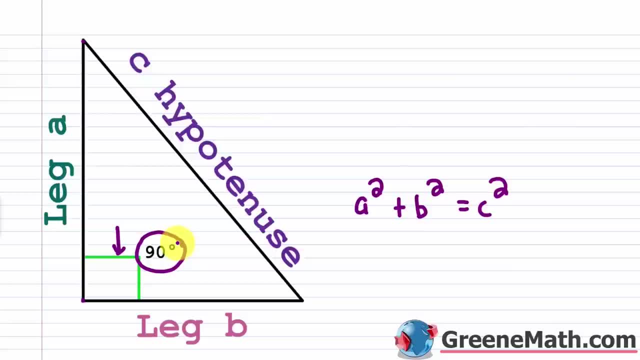 Okay, So this triangle has a 90 degree angle, Or a right angle. It is known as a right triangle. Okay, A right triangle. Now, with a right triangle, You have two shorter sides that are known as legs. So here you have this leg A. 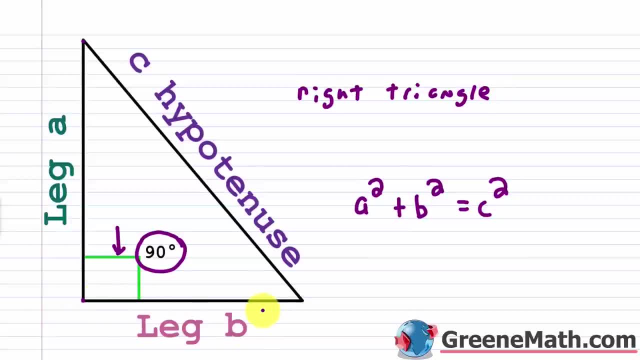 And this leg B. Okay, So those are the two shorter sides of the right triangle. Then the longest side Is always going to be opposite of the 90 degree angle. So opposite of that would be here. That's labeled as C. 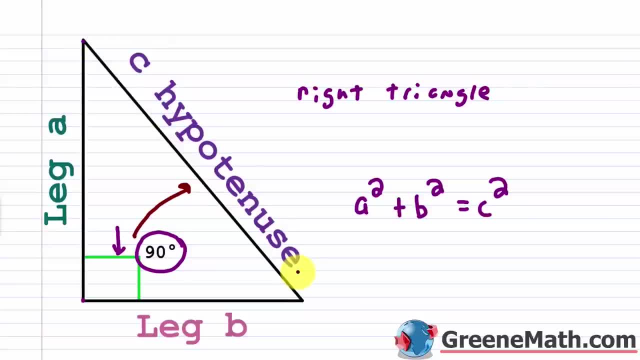 And it's known as the hypotenuse. Okay, So the way the Pythagorean formula works Is: it tells us that kind of the measure of leg A. So from here to here, If we square that, So that's where you get the A squared. 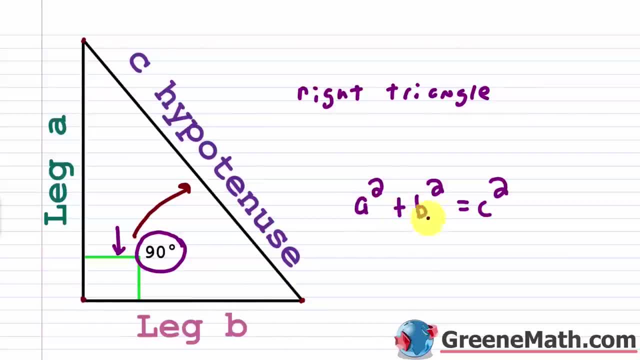 Then plus the measure of leg B, So from here to here. So you take that and you square it, So you're summing those two amounts together. So A squared plus B squared, This is equal to C or the hypotenuse squared. 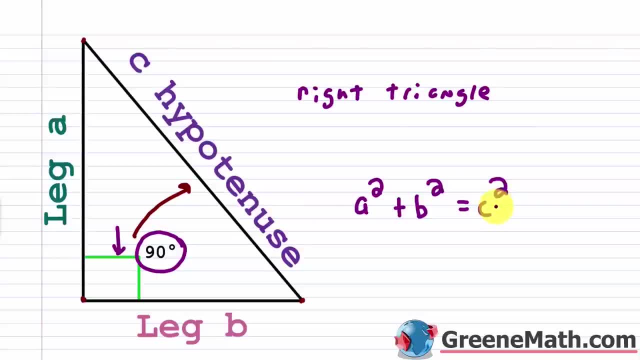 Okay, So this is true for any right triangle that you work with. What we're going to see Is that we can use this kind of Pythagorean formula To develop a distance formula That's going to tell us the distance Between two points on a coordinate plane. 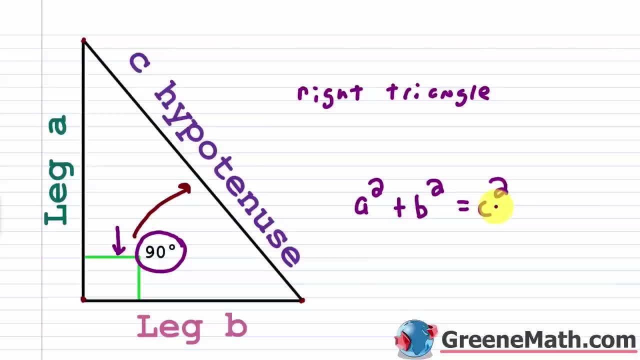 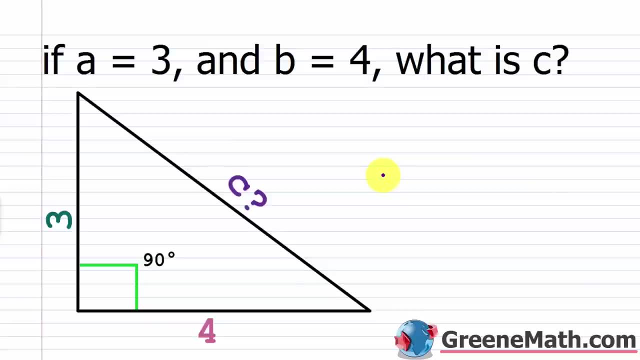 But before we jump into that, Let's look at a little sample problem, Just to get our feet wet. So when we're using our Pythagorean formula, If two of the three sides are known, We can solve for the third side that is unknown. 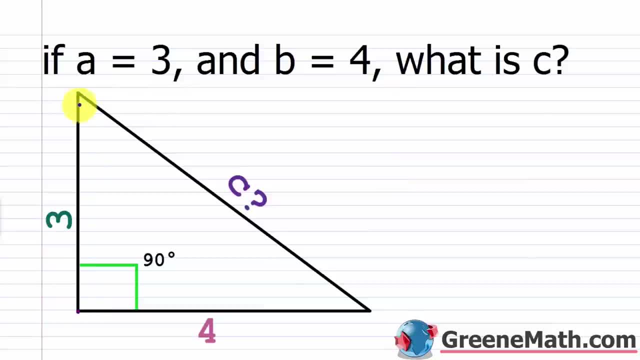 So in this case we're given that A is three, So that's going to be from here to here. Okay, that's my leg A. B is four, So that's going to be from here to here. So that's my leg B. 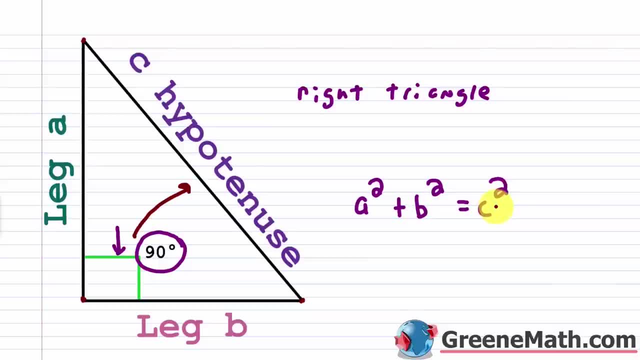 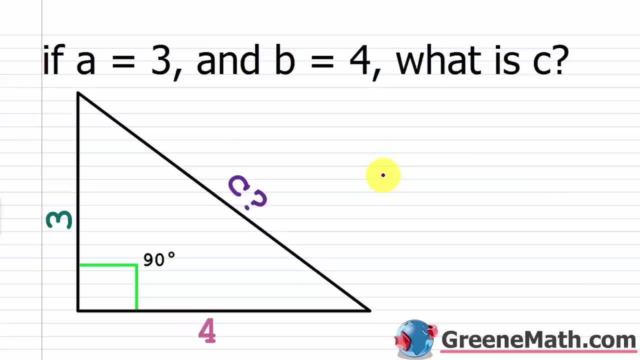 Now, what we're going to see is that we can use this kind of Pythagorean formula to develop a distance formula that's going to tell us the distance between two points on a coordinate plane. But before we jump into that, let's look at a little sample problem just to get our feet wet. So when we're using our Pythagorean formula, if two of the three sides are known, we can solve for the third side that is unknown. So in this case, we're given that A is three, so that's going to be from here to here, okay? That's my leg A. B is four, so that's going to be from here to here, okay? 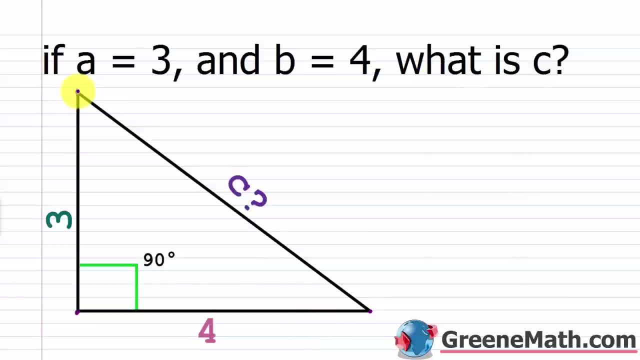 So that's my leg B. We want to know what is C. C is from here to here. That's our hypotenuse, 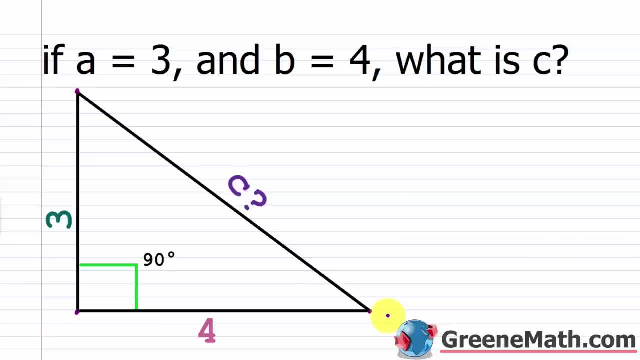 okay? So all I need to do is plug into my Pythagorean formula, and I can crank out an answer. So I have A squared plus B squared equals C squared, okay? Plug in for A. What is A? It's three, so just plug that in there. What is B? That's four, so just plug that in there. So three squared is nine, plus four squared is 16. This equals C squared. I'm going to flip this around just so I have my variable on the left side. So I'm going to say C squared equals nine plus 16 is 25. Okay, so we haven't solved something like this yet, and we're going to get to this as we kind of progress through our course. But essentially, what I want to do, if I want to isolate C, since it's being squared, I want to take the square root of each side, right? I'm always thinking about how can I undo what's being done to my variable, right? So since C, the variable I'm trying to solve for is being squared, to undo that, I just take the square root, okay? And to make it legal, I've got to take the square root of each side. So let me kind of scooch this down just a little bit. So I would take the square root of this side and the square root of this side. 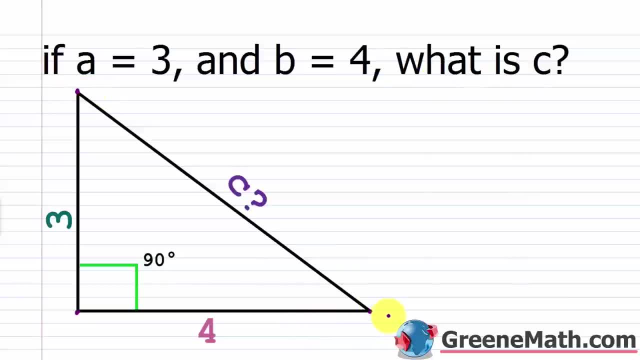 We want to know what is C? C is from here to here. That's our hypotenuse. So all I need to do is plug into my Pythagorean formula And I can crank out an answer. So I have A squared plus B squared. 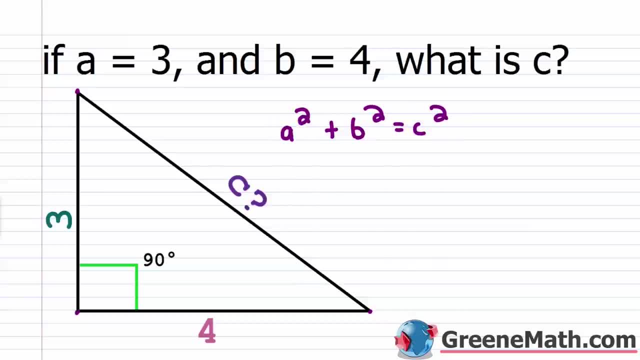 Equals C squared. Plug in for A. What is A, It's three, So just plug that in there. What is B, That's four, So just plug that in there. So three squared is nine Plus four squared is sixteen. 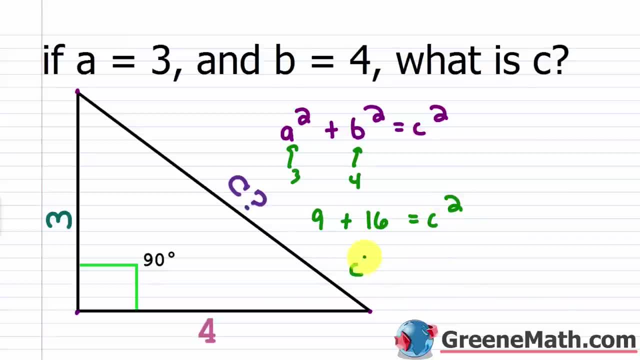 So I'm going to turn this around, Just so. I have my variable on the left side. So I'm going to say: C squared equals Nine plus sixteen is twenty-five. Okay, so we haven't solved something like this yet, And we're going to get to this as we kind of progress through our course. 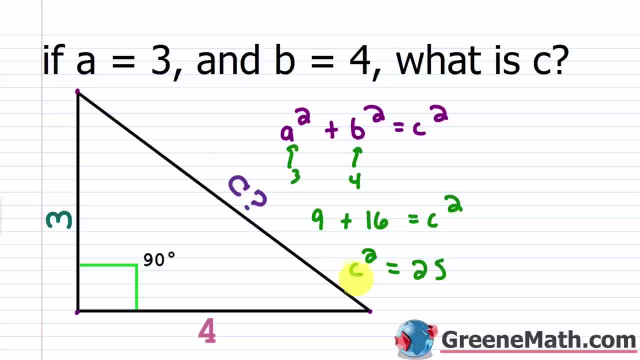 And we're going to get to this as we kind of progress through our course. But essentially what I want to do, If I want to isolate C, Since it's being squared, I want to take the square root of each side. I'm always thinking about how can I undo? 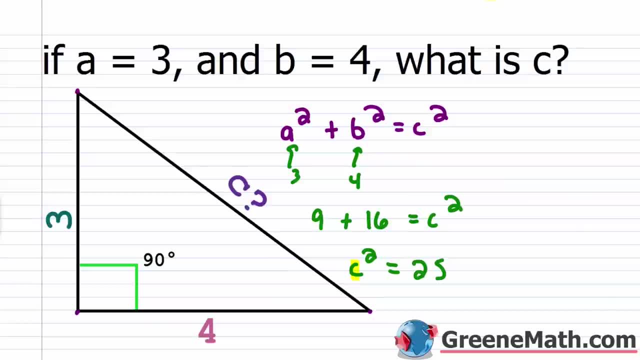 What's being done to my variable Right. So the variable I'm trying to solve for is being squared. To undo that, I just take the square root. Okay, And to make it legal, I've got to take the square root of each side. 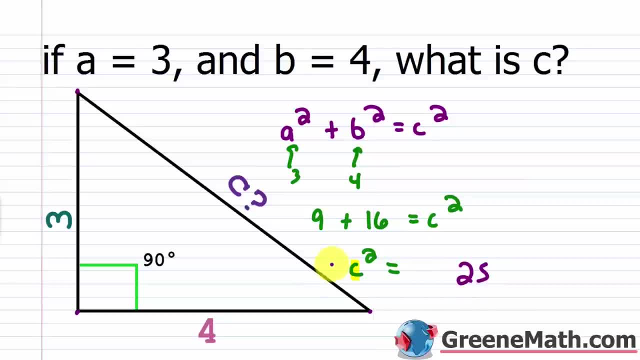 So let me kind of scooch this down just a little bit. So I would take the square root of this side And the square root of this side. Now, In most cases when you do this, You want to go plus or minus over here. 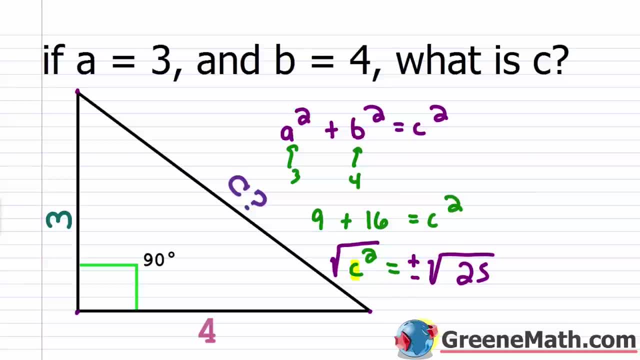 Okay, In this case you're not going to, And I'll explain why in a second. First, let's kind of solve, just given the way that I've presented it here. So this index of two, Right, Remember, this square root has an index of two. 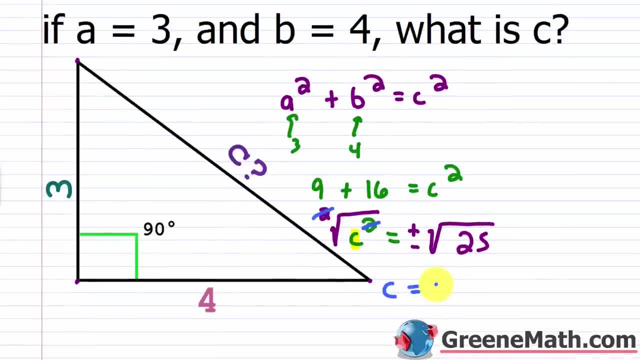 Is going to cancel with this exponent of two. Okay, So I now have C by itself And it's equal to plus or minus the square root of twenty five, Which is five. Now, Does that make sense? Well, remember if I erase all this. 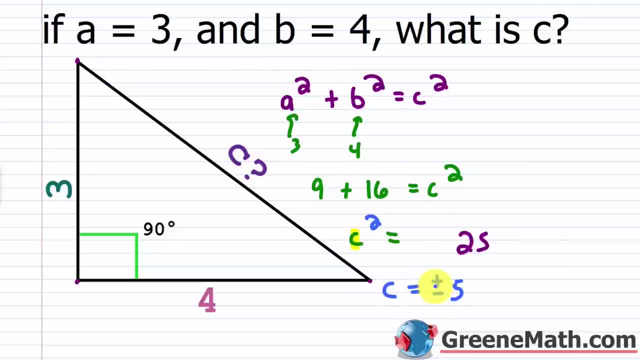 And I bring this back to C: squared equals twenty five. Well, C could be five Right Five squared is twenty five, And C could also be negative five. That's important, But for now we just take it as a given. But we need to understand that here, in this specific situation, 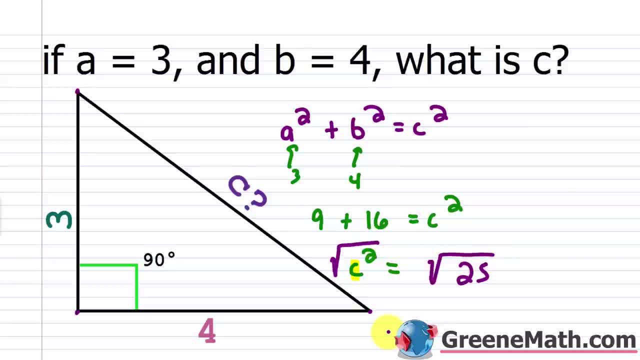 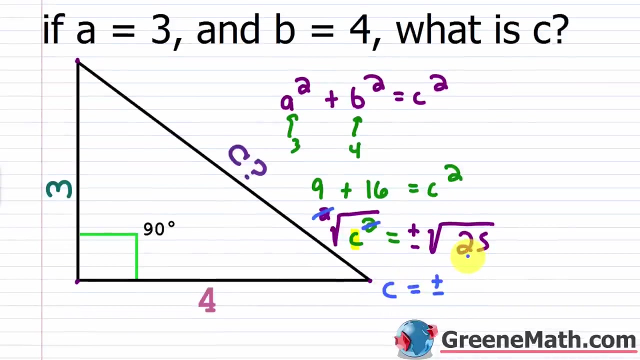 Now, in most cases, when you do this, you want to go plus or minus over here, okay? In this case, you're not going to, and I'll explain why in a second. First, let's kind of solve just given the way that I've presented it here. So this index of two, right? Remember, this square root has an exponent of two, okay? So I now have C by itself, and it's equal to plus or minus the square root of 25, which is five. Now, does that make sense? Well, remember, if I erase all this, and I bring this back to C squared equals 25, well, C could be five, right? Five squared is 25. And C could also be negative five, right? Negative five squared is 25. So that's why you have that little plus or minus there. And we'll get to that later on in the course as to why that's important. But for now, we just take it as a given. 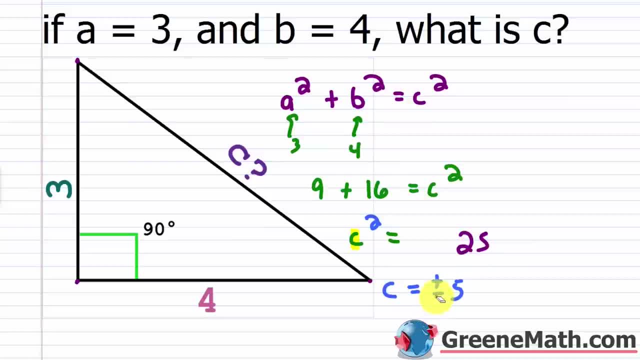 But we need to understand that here in this specific situation, I don't need a negative five as an answer. I only need the principal square root when I do this, because five is my only valid solution. Why? Because I'm thinking about how far is it from here to here? I'm basically thinking about the distance for the measure of C, and that's not going to be negative, 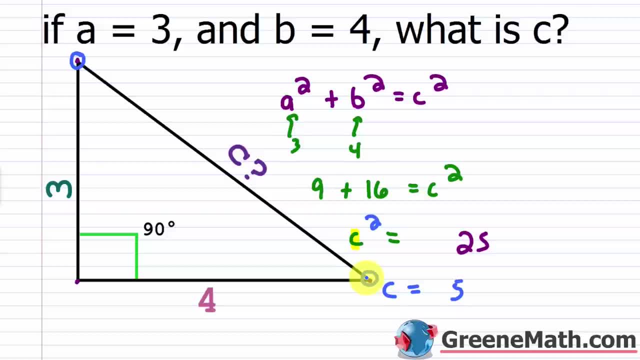 right? Negative five is a nonsensical answer. It can only be positive five, okay? So we've seen an example of working with the Pythagorean formula, and now we're going to use it to find the distance 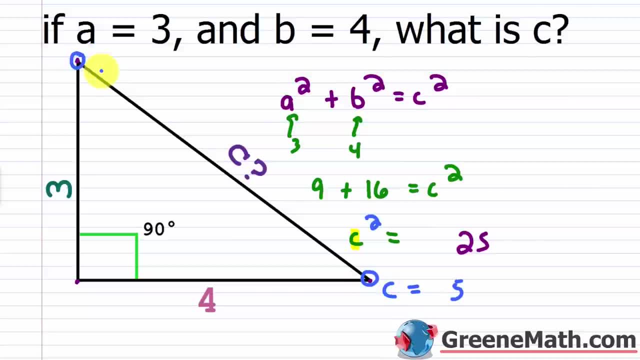 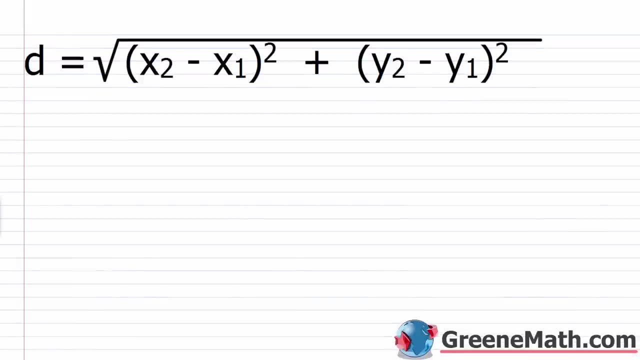 for the coordinate plane. Essentially, you're going to have a point that's here and here, okay? And what we're going to do is we're going to derive a formula that lets us solve for the unknown, which is going to be the hypotenuse, given the fact that we're going to be able to find this horizontal distance here and this vertical distance here. So what we have on the screen here is our distance formula. Again, the distance formula is just allowing us to easily calculate the distance between two points in a coordinate plane. It's a direct application of what we're just looking at. Again, the Pythagorean formula. 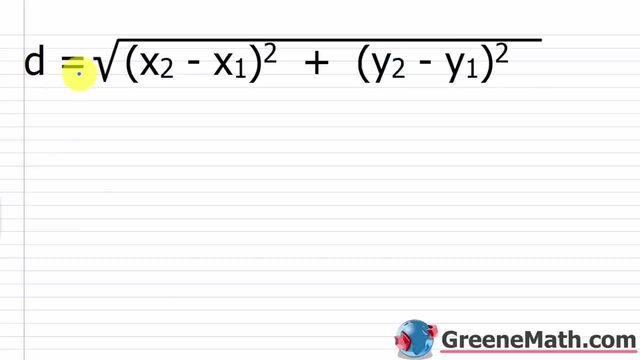 So what we see here is that d, which stands for distance, is equal to the square root of, we have x sub 2 minus x sub 1 squared, plus we have y sub 2 minus y sub 1 squared. 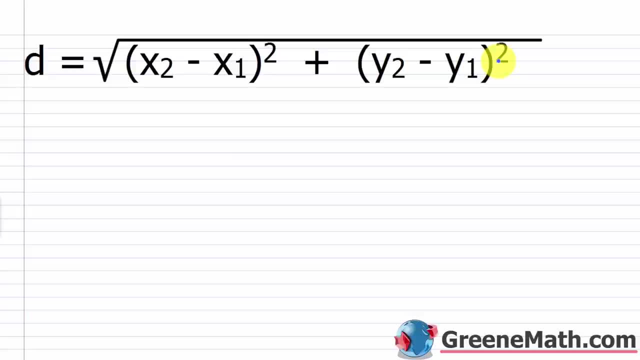 And again, just like when we worked with slope, okay, we can label one of our points as x sub 1, y sub 1, the other as x sub 2, y sub 2. It's not going to matter which is labeled as which. 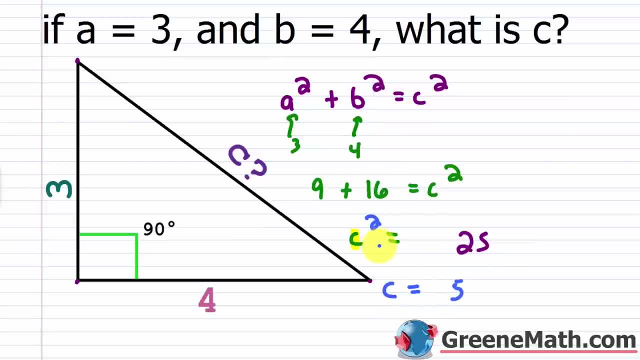 I don't need a negative five as an answer. I only need the principal square root. when I do this? Because five is my only valid solution. Why? Because I'm thinking about how far is it from here to here. I'm basically thinking about the distance for the measure of C. 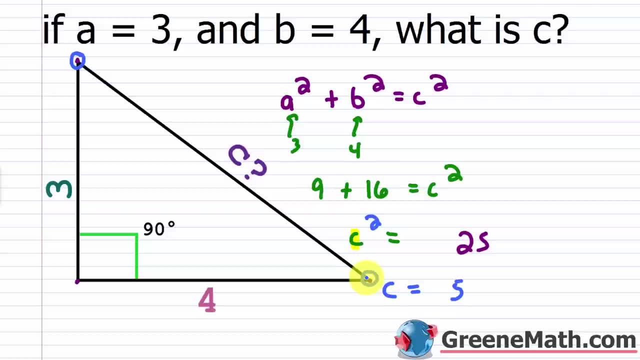 And that's not going to be negative Right? Negative five is a nonsensical answer. It can only be positive five. Okay, So that's the Pythagorean formula, And now we're going to use it to find the distance between two points in a coordinate plane. 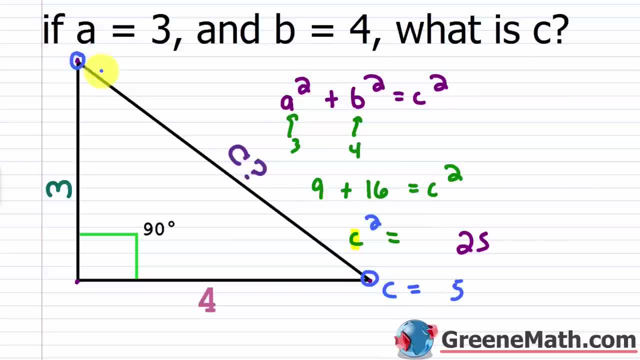 Essentially, You're going to have a point that's here and here, Okay, And what we're going to do is we're going to derive a formula That lets us solve for the unknown, Which is going to be the hypotenuse. 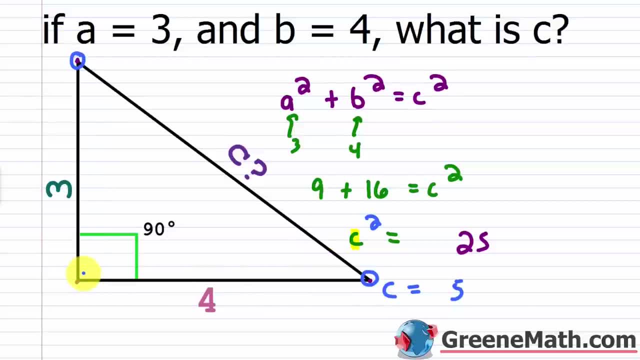 Given the fact that we're going to be able to find this horizontal distance here And this vertical distance here. So what we have on the screen here Is our distance formula. Again, the distance formula is just allowing us to easily calculate the distance between two points in a coordinate plane. 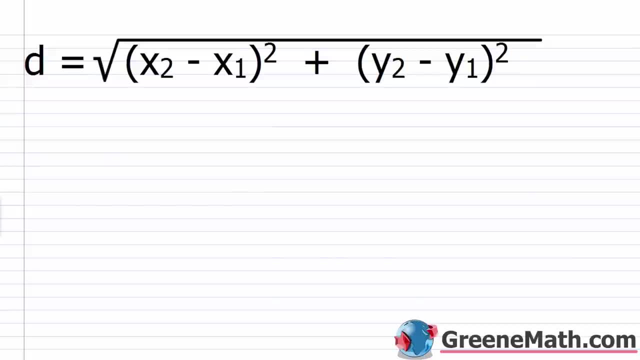 Is our distance formula. Again, the distance formula is just allowing us to easily calculate the distance between two points in a coordinate plane. It's a direct application of what we're just looking at Again, the Pythagorean formula. So what we see here is that d 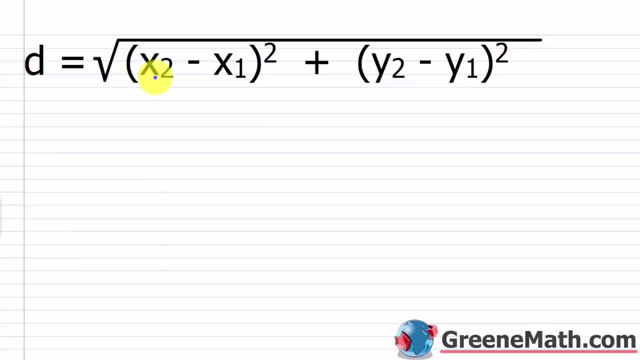 Which stands for distance, Is equal to the square root of. We have x sub two minus x sub one, squared. Plus we have y sub two minus y sub one, squared. And again, Just like when we worked with slope, Okay, We can label one of our points as x sub one, y sub one. 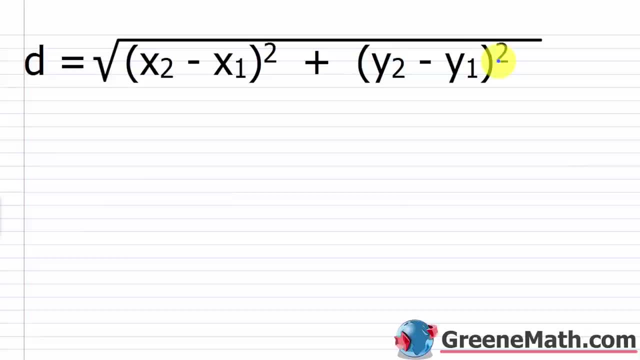 The other as x sub two, y sub two. It's not going to matter which is labeled as which. You're going to get the same answer either way. So how does this relate to the Pythagorean formula? So how does this relate to the Pythagorean formula? 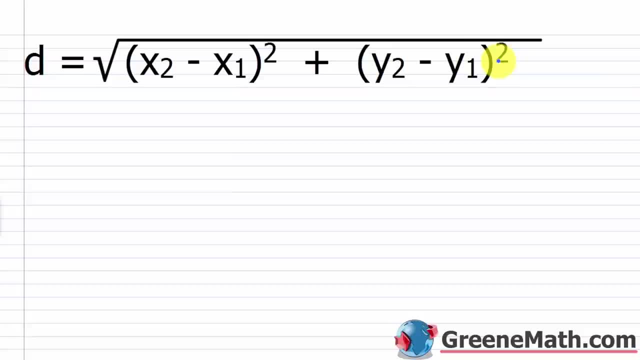 Well, let's look at an example and work through that completely, And then we'll kind of bust through a bunch of examples, Alright, So we want to find the distance between each pair of points And we're going to start out with five comma negative two. 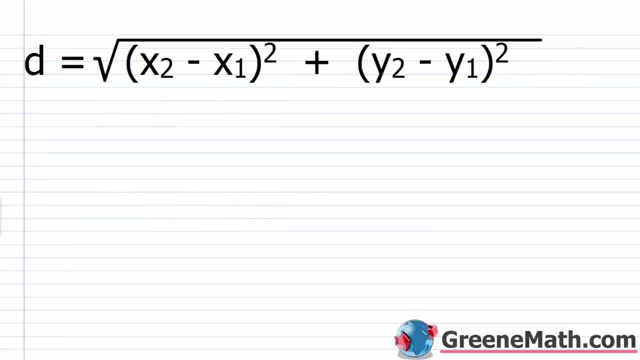 And negative seven comma negative seven. So let me go back up. So we have five comma negative two And we have negative seven comma negative seven, And we have negative seven comma negative seven. So the first thing I'm going to do is just plug into the formula. 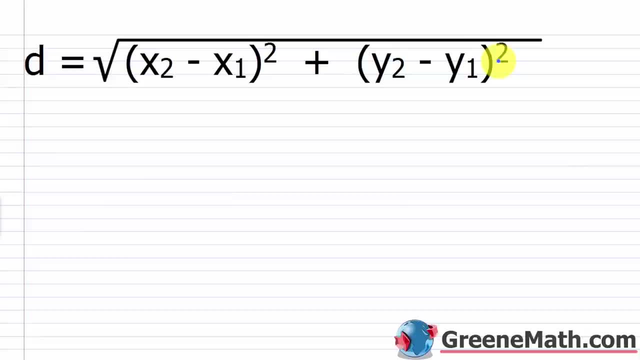 You're going to get the same answer either way. So how does this relate to the Pythagorean formula? Well, let's look at an example and work through that completely. 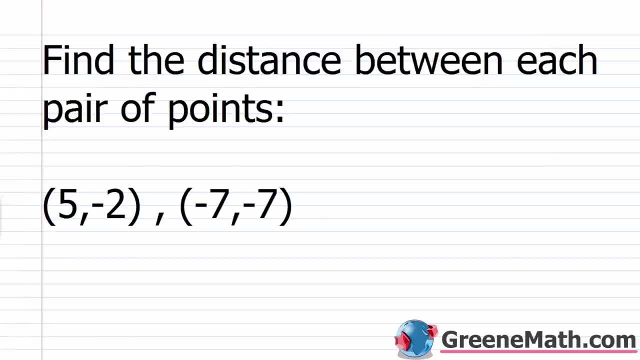 And then we'll kind of bust through a bunch of examples. All right, so we want to find the distance between each pair of points. 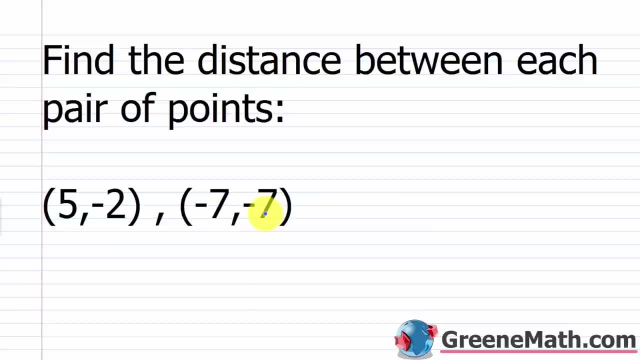 And we're going to start out with 5 comma negative 2 and negative 7 comma negative 7. 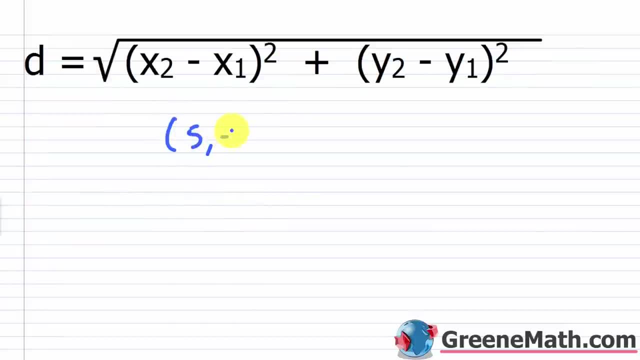 So let me go back up. So we have 5 comma negative 2, and we have negative 7 comma negative 7. So the first thing I'm going to do is just plug into the formula. We're going to get an answer. Then we're going to go to the coordinate plane. I'm going to show you where this comes from. So d, the distance, is equal to the square root of. So I'm going to label this guy as x sub 1, y sub 1, and I'll label this as x sub 2, y sub 2. Again, you can change that up. It wouldn't matter. So x sub 2 is going to be negative 7. Just plug in that in for x sub 2 there. Then minus x sub 1 is going to be 5. Just plug in that in there. This is squared. Then plus, we've got y sub 2, which is negative 7. Just plug in that in for y sub 2 there. 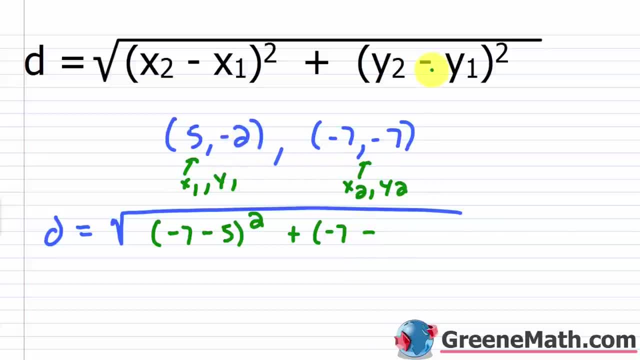 Then minus y sub 1, which is negative 2. Be careful. You're going to have minus a negative, which is plus a positive. So this is going to be plus. 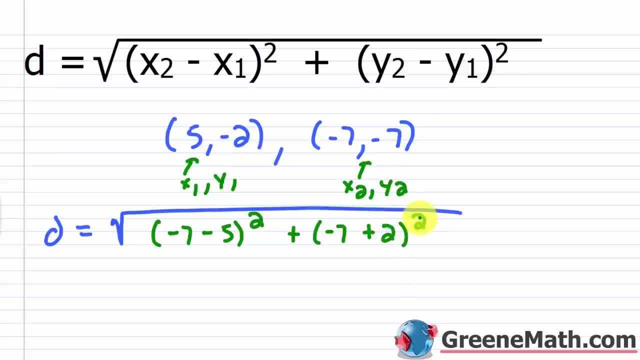 And then this guy is squared. So all I did was I plugged in. Nothing fancy there. 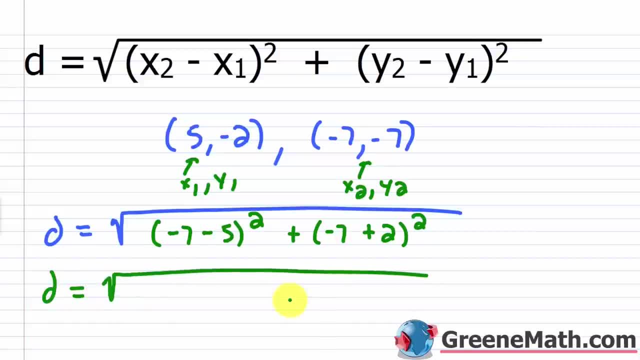 So my distance, d, is going to be equal to the square root of. All I've got to do is just kind of crank this out. Negative 7 minus 5 is going to be negative 12. Negative 12 squared is 144. Then plus, negative 7 plus 2 is going to be negative 5. Negative 5 squared is 25. 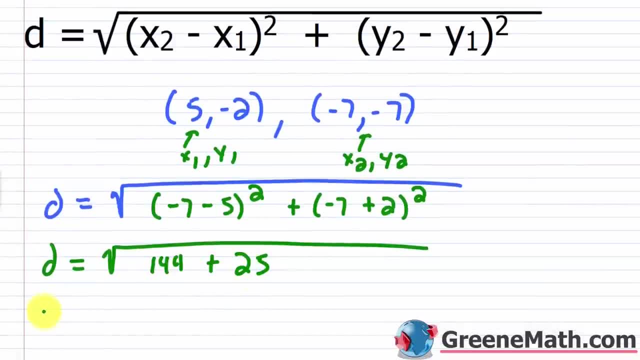 So 144 plus 25 is 169. So d, my distance, is going to be equal to. The square root of 169, which is basically 13, right? 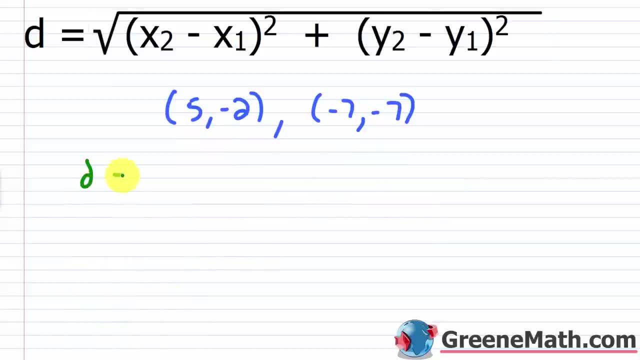 So let me kind of erase this and I'll say the distance between the two points is going to be 13. 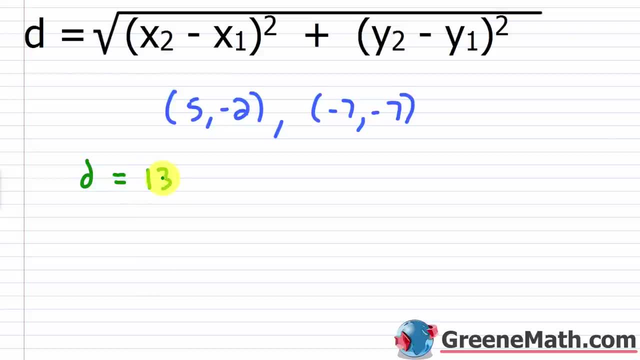 Okay, so where did this come from? I know most of you just want to be able to get through your homework. So once you have the formula, you're basically good to go. 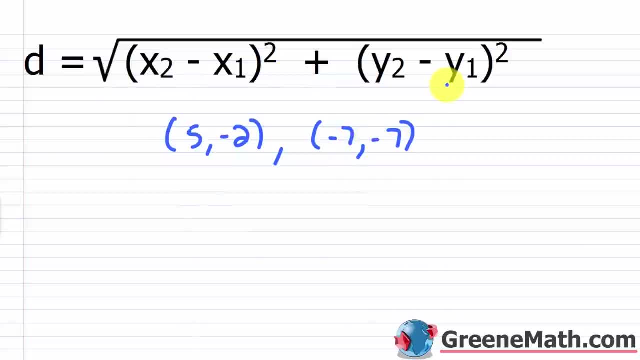 We're going to get an answer. Then we're going to go to the coordinate plane from. so d the distance is equal to the square root of, so i'm going to label this guy as x sub 1, y sub 1, and i'll label this as x sub 2, y sub 2 again. you can change that up, it wouldn't matter. so x sub 2. 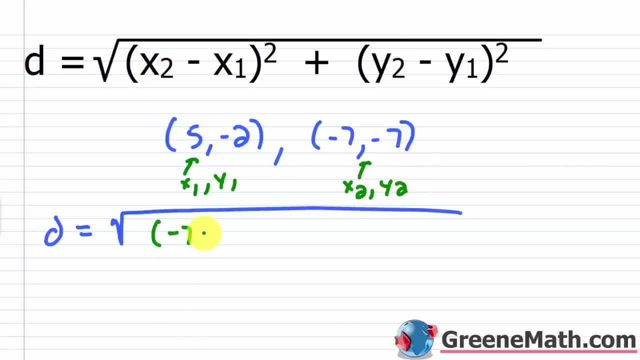 is going to be negative 7. just plugging that in for x sub 2 there. then minus x sub 1 is going to be 5. just plugging that in there, this is squared. then plus we've got y sub 2, which is negative 7. 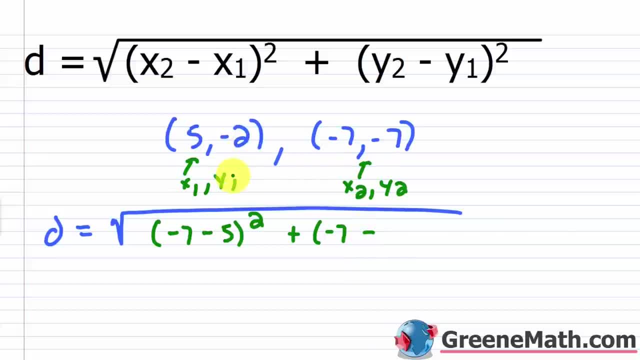 just plugging that in for y sub 2 there, then minus y sub 1, which is negative 2. be careful, you're going to have minus a negative which is plus a positive, so this is going to be plus 2, and then this guy is squared. so all i did was i plugged in. okay, nothing's. 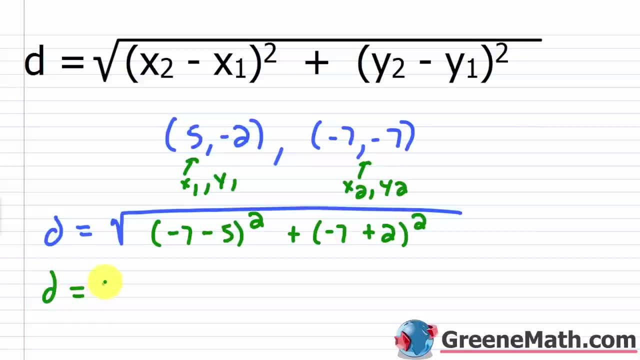 nothing fancy there. so my distance d is going to be equal to the square root of. all i'm going to do is just kind of crank this out: negative 7 minus 5 is going to be negative 12. negative 12 square is 144.. then plus negative 7 plus 2 is going to be negative 5. 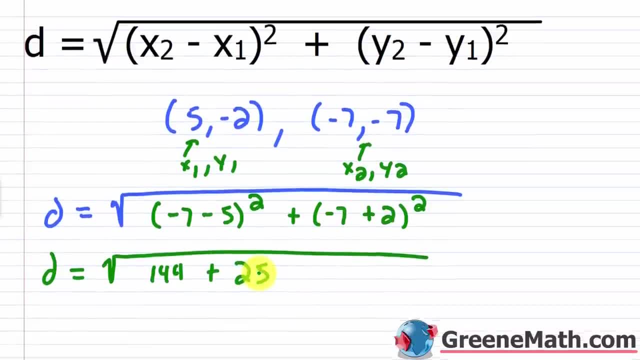 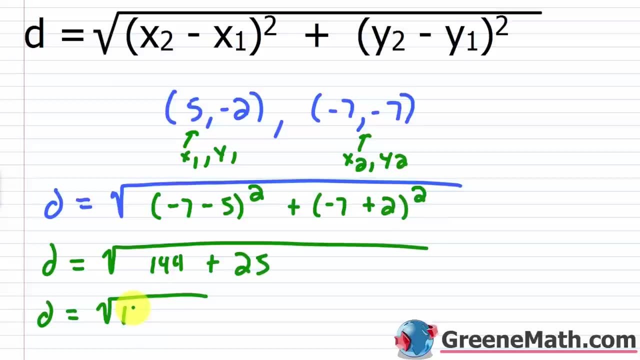 negative. 5 squared is 25, so 144 plus 25 is 169, so d my distance is going to be equal to the square root of 169, which is basically 13, right? so let me kind of erase this and i'll say the distance between: 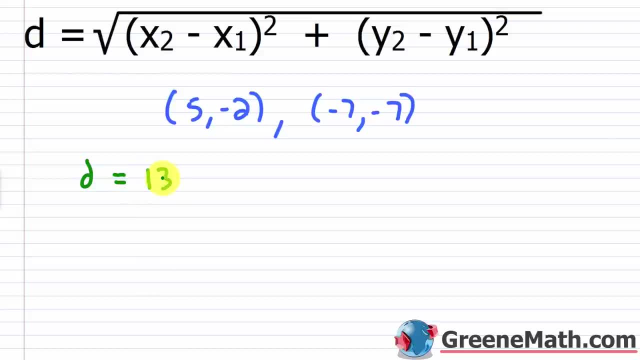 the two points is going to be 13. okay, so where did this come from? i know most of you just want to be able to get through your homework, so once you have the formula, you're basically good to go. you can just plug in. but i want you to understand where it came from. so let's go to the coordinate. 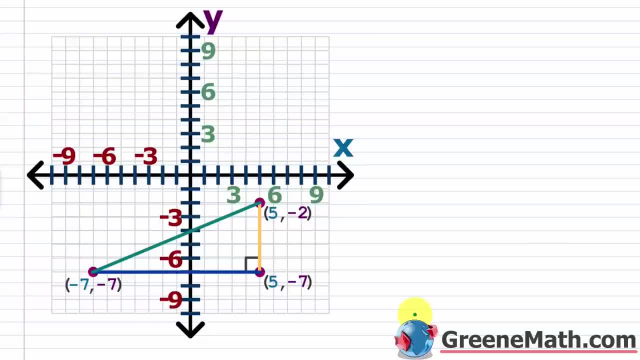 plane. let's think about the distance between the two points, kind of using a different approach. so again we had five comma negative two, and we also had negative seven comma negative seven. so i've kind of pre-drawn everything to make this a little faster. so we have five comma negative two. 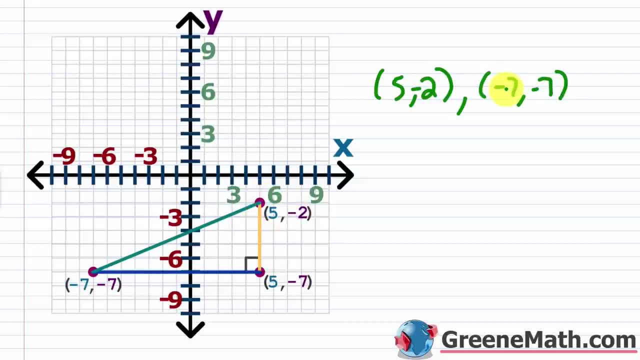 that's right here. okay, that's your five negative two and you have negative seven, comma negative seven. so that's going to be right here. so you'll notice that i drew in an extra point to kind of form the right triangle. so the way i did that was i took the x coordinate. 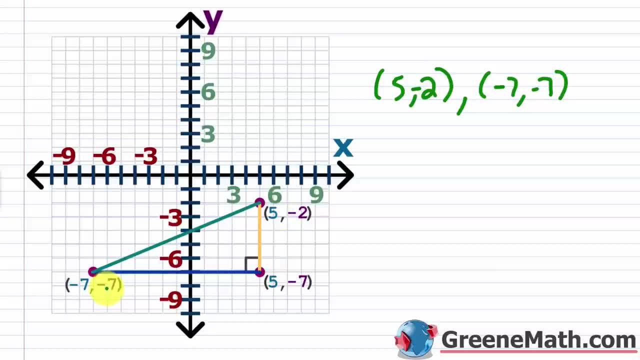 four, and i drew in an extra point, and i drew in an extra point, and i drew in an extra point from here, which was five, and i took the y coordinate from here, which was negative seven. that gave me my third vertex so i could again draw the right triangle. so what i can see is that i can 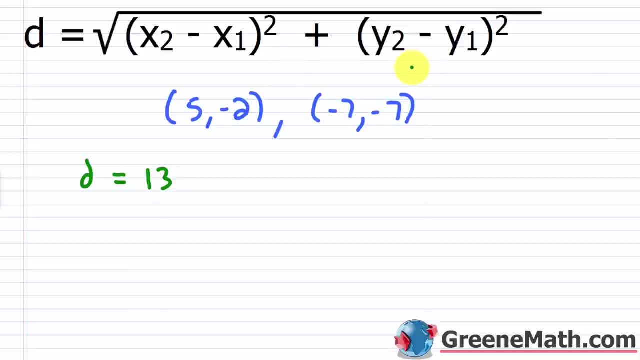 You can just plug in, but I want you to understand where it came from. So let's go to the coordinate plane. 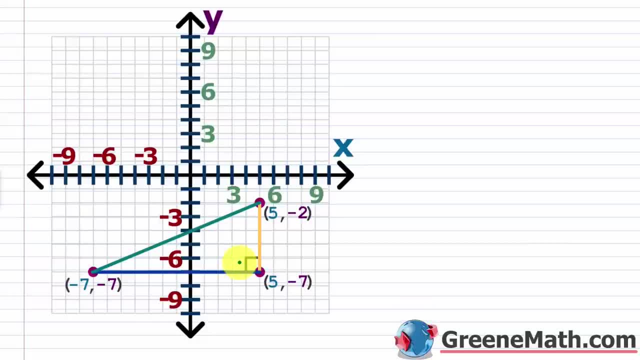 Let's think about the distance between the two points kind of using a different approach. So again, we had 5 comma negative 2 and we also had negative 7 comma negative 7. 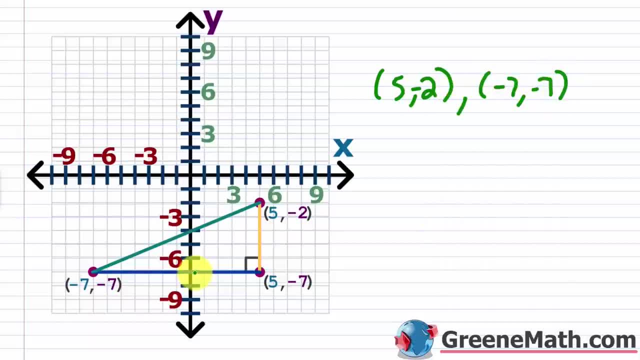 So I've kind of pre-drawn everything to make this a little faster. So we have 5 comma negative 2. That's right here. Okay, that's your 5 negative 2. And then you have negative 7 comma negative 7. So that's going to be right here. So you'll notice that I drew in an extra point to kind of form the right triangle. So the way I did that was I took the x coordinate from here, which was 5. And I took the y coordinate from here, which was negative 7. That gave me my third vertex. 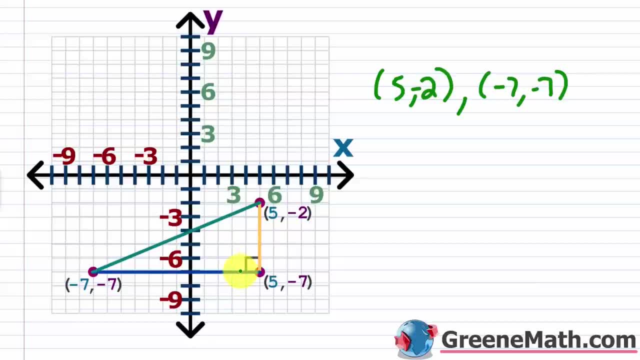 So I can again draw the right triangle. So what I can see is that I can find the measure from here to here. That's going to be a vertical leg for me. That's going to be my leg A. I can find the measure from here to here. That's going to be my horizontal leg or my leg B. Okay, and all I need to solve for is this C, which is the distance between these two points. That's my unknown. Okay, so how do I find the measure for leg A? Well, since this is a vertical line, I'm just thinking about y values. Okay, because it's parallel to the y axis. 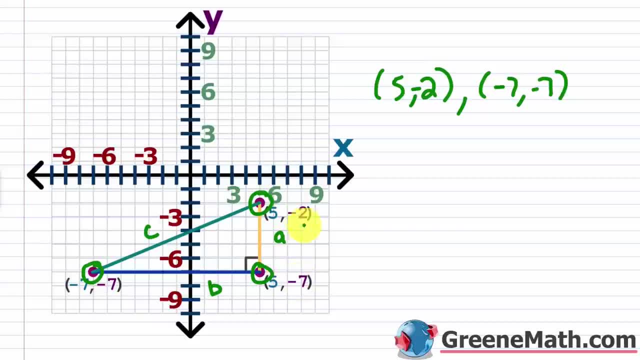 So how far do I move from this y coordinate here of negative 7 to this y coordinate here of negative 2? Well, most of you would realize that you just need to subtract the y values. 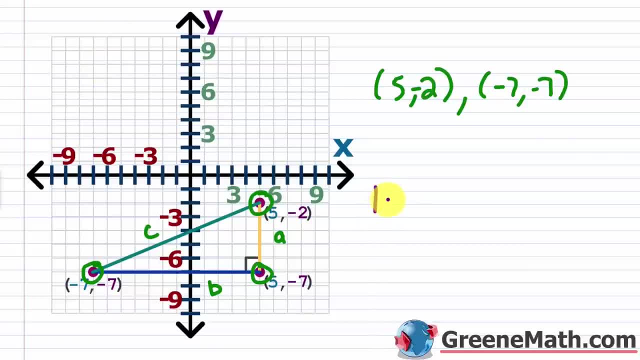 Right? So you would just basically do inside of absolute value bars, negative 2 minus a negative 7 which would be equal to what? It would be the absolute value of negative 2 plus 7 which would be equal to the absolute value of 5, which is 5. 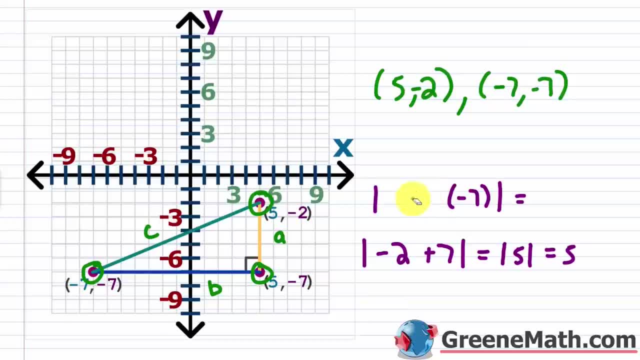 You could also do it. the other way because you use absolute value. So I could reverse this completely. And I could say that we had negative seven minus a negative two. Okay. You get the same answer. So negative seven minus a negative two inside of absolute value bars would be the absolute value of negative seven plus two, which would be the absolute value of negative five, which would be five. Okay. 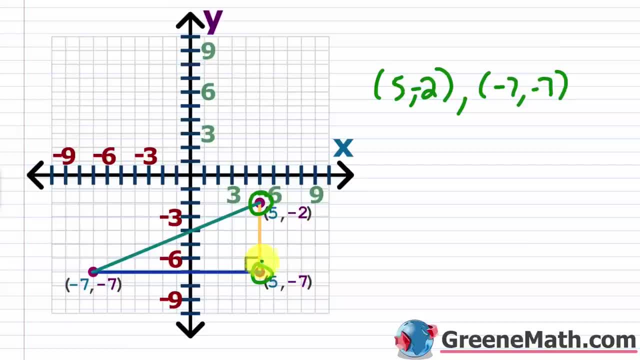 find the measure from here to here that's going to be a vertical leg for me, that's going to be my leg a. i can find the measure from here to here that's going to be my horizontal leg or my leg b. okay, and all i need to solve for is this c, which is the distance between these two points, that's. 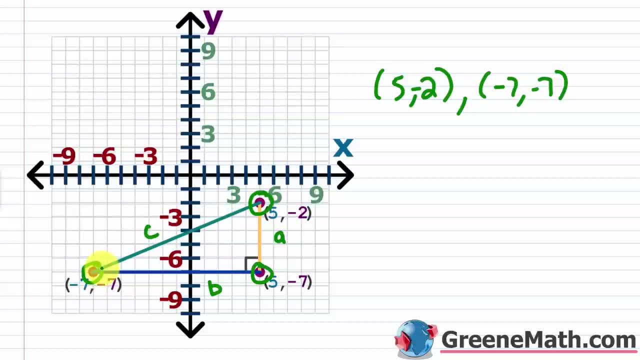 my unknown. okay, so how do i find the measure for leg a? well, since this is a vertical line, i'm just thinking about y values. okay, because it's parallel to the y axis. so how far do i move from this y coordinate here of negative seven to this y coordinate here of negative two? well, most of. 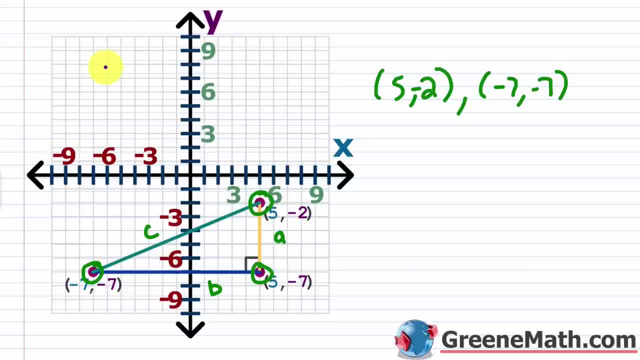 you would realize that you just need to subtract the y values, right, so you would just basically do, inside of absolute value bars, negative two minus a negative seven, which would be equal to what would be the absolute value of negative two plus seven, which would be equal to the absolute value. 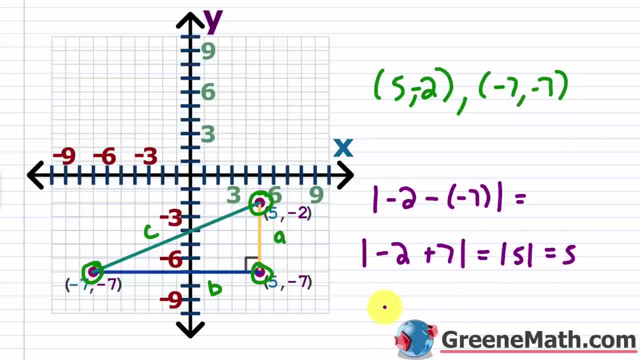 of five, which is five. you could also do it the other way, because you use absolute value, so i could reverse this completely and i could say that we had negative seven minus a negative two. okay, you get the same answer. so negative seven minus a negative two inside of absolute value. 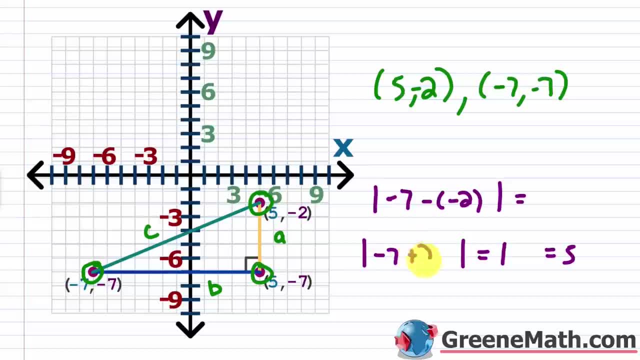 bars would be the absolute value of negative. seven plus two, which would be the absolute value, are using absolute value. we're using absolute value because we're calculating a distance. we don't want to end up with a negative value. Okay, so notice how we just found the difference. 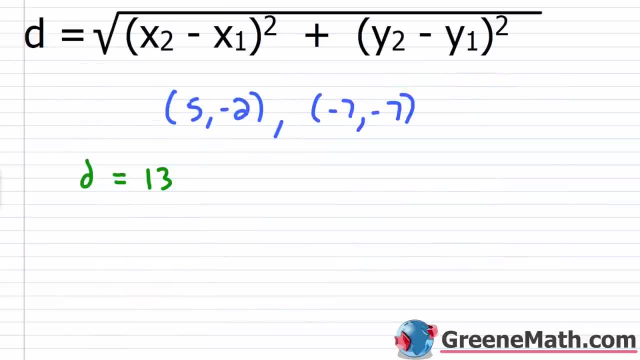 in y values. Now, if we go back up, you'll notice that when we did our formula, we have y sub two minus y sub one. we're just calculating the difference in y value. So we're doing the same thing. We don't have absolute value bars because we're squaring the result. Okay, so if you square, 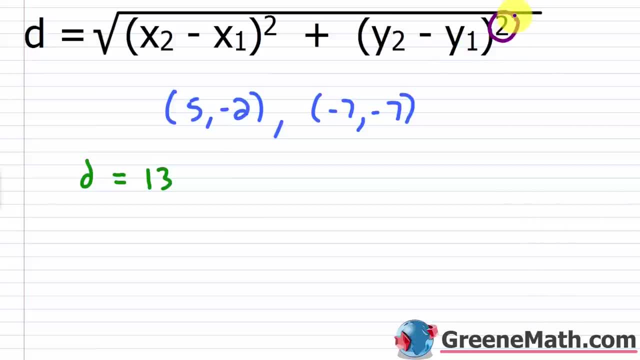 something that's negative. if I ended up with negative five and I squared, I get 25.. If I end up with five and I square, to get 25.. So I don't need absolute value bars. So that's why they're. 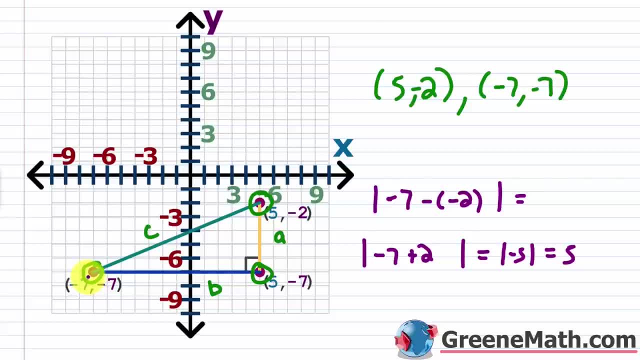 not there. The same thing is going to go when I find the kind of horizontal legs measure. So now I'm dealing with a horizontal line which is going to be parallel to the x axis, So I'm thinking about x values now. So I have an x value of negative seven and I have an x value of five. 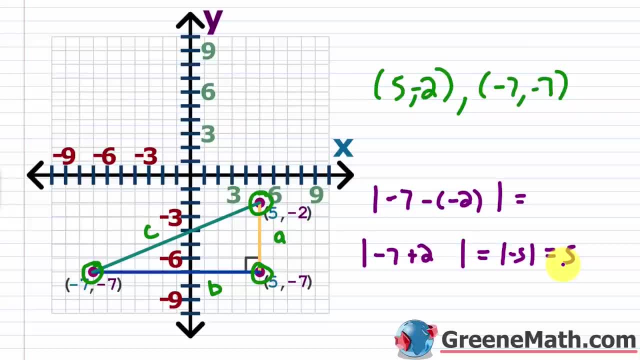 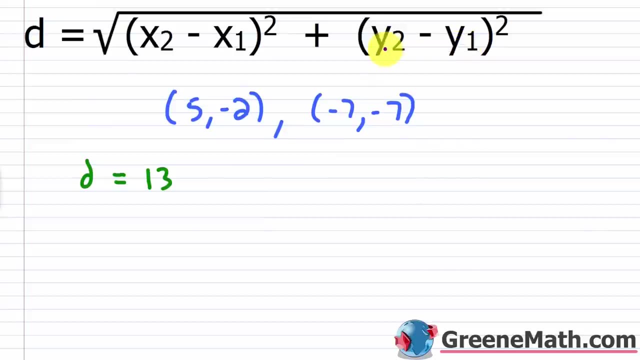 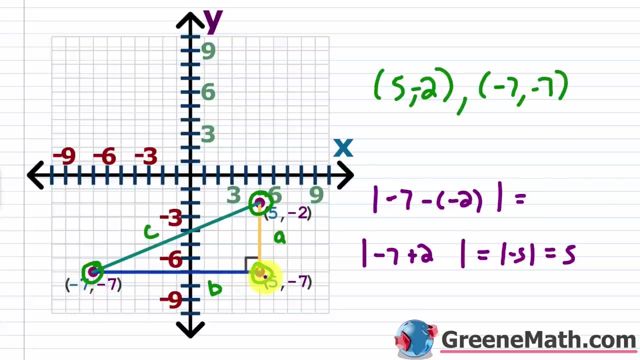 Now you might say, well, why are you using absolute value? We're using absolute value because we're calculating a distance. We don't want to end up with a negative value. Okay. So notice how we just found the difference in Y values. Now, if we go back up, you'll notice that when we did our formula, we have Y sub two minus Y sub one. We're just calculating the difference in Y values. So we're doing the same thing. We don't have absolute value bars because we're squaring the result. Okay. So if you square something that's negative, if I ended up with negative five and I squared, I get 25. If I end up with five and I squared, I get 25. So I don't need absolute value bars. So that's why they're not there. The same thing is going to go when I find the kind of horizontal legs measure. 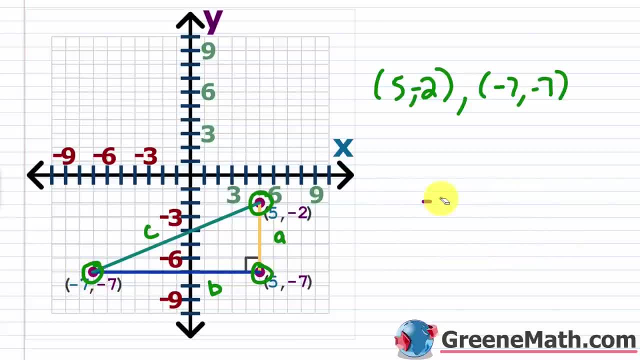 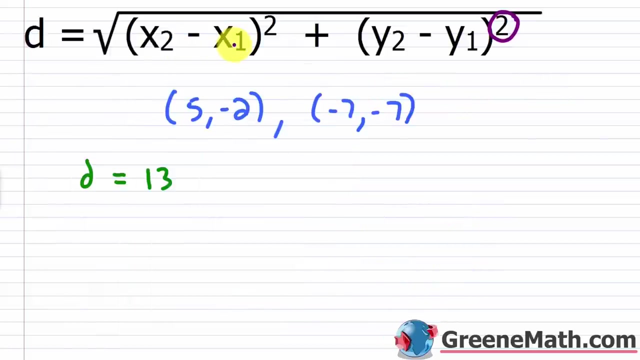 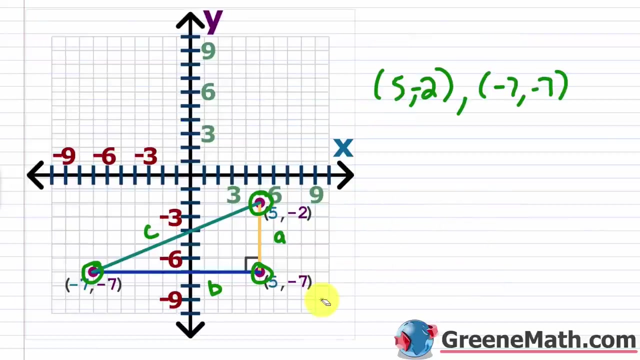 So now I'm dealing with a horizontal line, which is going to be parallel to the X axis. So I'm thinking about X values now. So I have an X value of negative seven and I have an X value of five. So I can either do the absolute value of five minus a negative seven, or I could do the absolute value of negative seven minus five. Gives me the same answer either way. So this would be equal to one. This would be equal to the absolute value of five plus seven, which is 12. So the absolute value of 12 is 12. Okay. So again, if I go back up, I can see that I have an absolute value of five. So I'm looking for the difference in X values. And again, if it's negative 12 and I squared, I get 144. If it's positive 12 and I squared, I get 144. So I don't need absolute value bars in that case. Okay. So once we know that leg A's measure is five and leg B's measure is 12, well, then I can plug into my formula, right? So I can say that this is A. So five is A and we're squaring that. Plus the B is going to be what? It's 12. So I can plug into my formula. 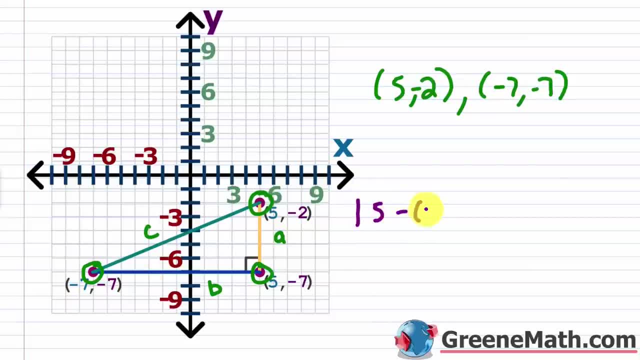 So I can either do the absolute value of five minus a negative seven or I could do the absolute value of negative seven minus five gives me the same answer either way. So this would be equal to what? this would be equal to the absolute value of five plus seven. 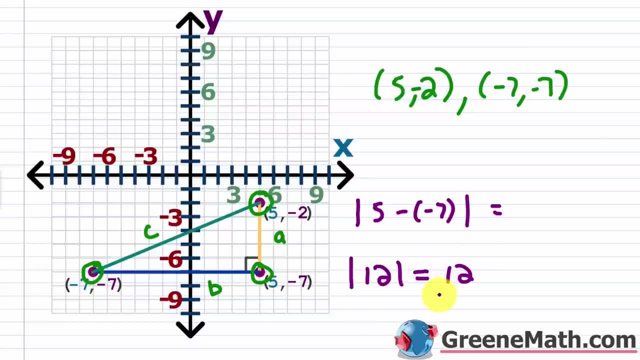 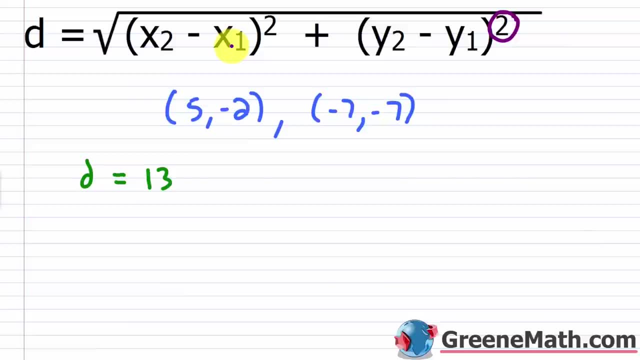 which is 12.. So the absolute value of 12 is 12.. Okay, So again, if I go back up, I'm looking for the difference in x values, And again, if it's negative, 12, and I square to get 144, if it's. 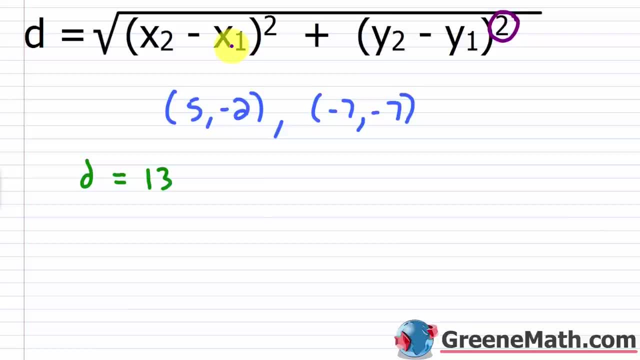 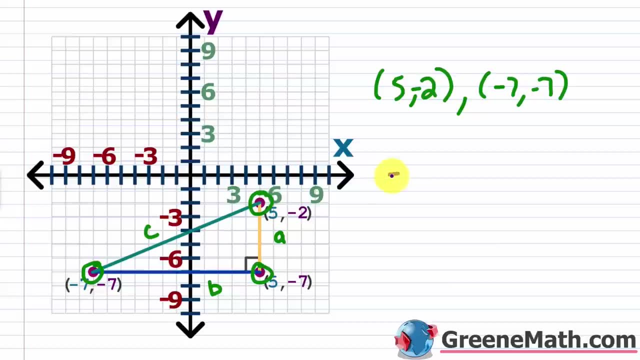 positive 12, and I square to get 144.. So I don't need absolute value bars in that case. Okay, So once we know that leg A's measure is five and leg B's measure is 12,, well then I can do the. 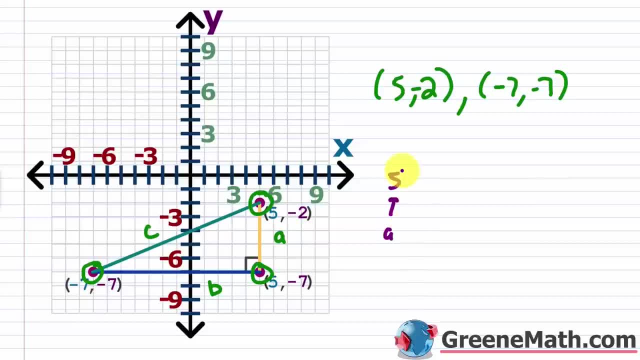 plug into my formula right. So I can say that this is A, So five is A, and we're squaring that plus the B is going to be what It's: 12.. So we're squaring that This is equal to C squared Okay. 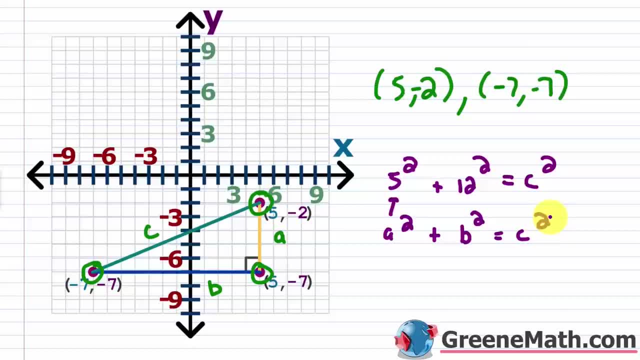 C squared, And in this case we just relabeled C with D for distance. That's all we did, So let's just label this as D. It doesn't matter, We're just changing the variables letter, but it means the same thing. Okay, So if I have D squared equals five squared. 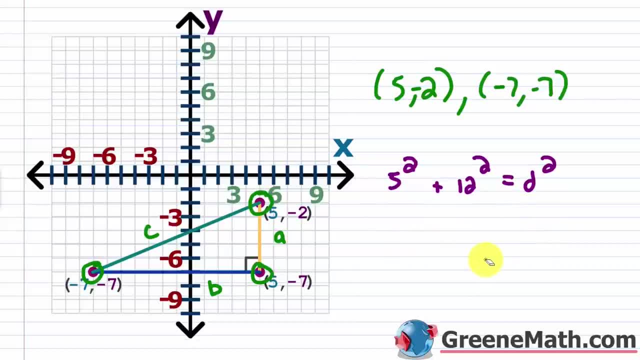 plus 12 squared. how do I solve for D? Well, at this point I could just take the square root of each side, right? I know I can simplify this further, but all I'm doing up here if I go back. 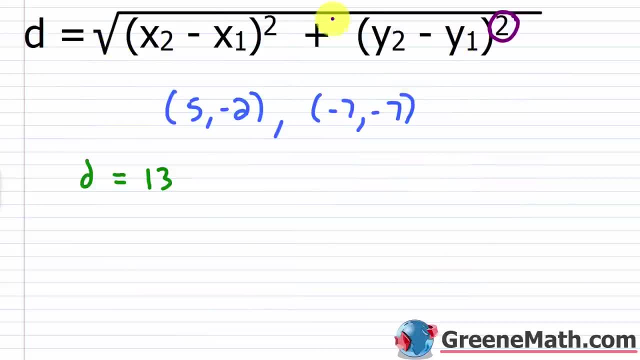 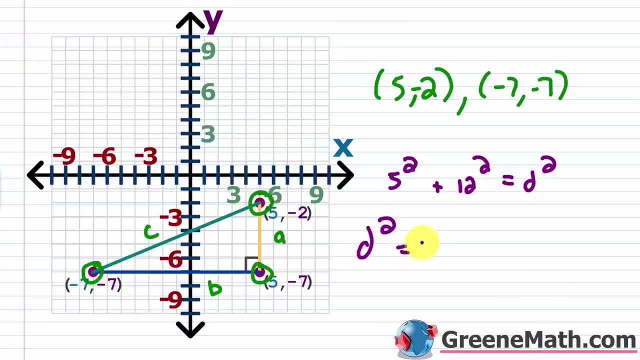 to my formula. once I have this guy, I can just take the square root of each side and I've solved for D. Okay, Let me go back down and make that crystal clear. So D squared equals you have five squared plus 12 squared. If I take the square root of each side, then this would go away and I have 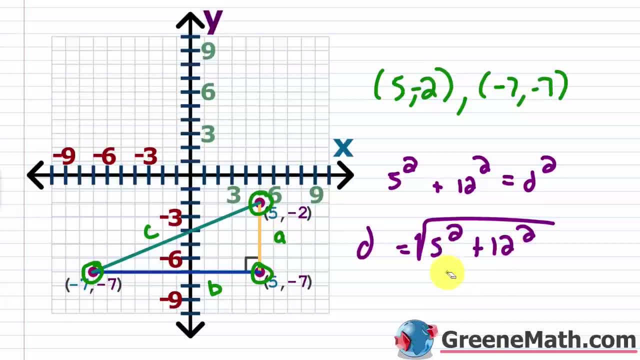 the square root of this, Then I could just calculate the square root of each side, and I could just calculate this: Five squared is 25, and 12 squared is 144, and then 25 plus 144 is 169.. And we all know. 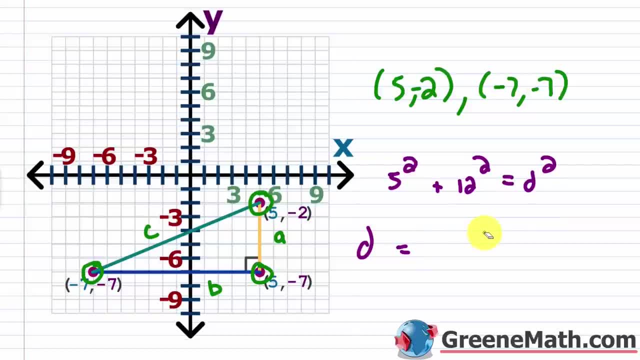 the answer from earlier. D equals square root of 169,, which is 13.. Okay, So just a quick insight into where this comes from. It's a direct application of the Pythagorean formula. I know most of you you know you're more interested in just being able to kind of get the formula and 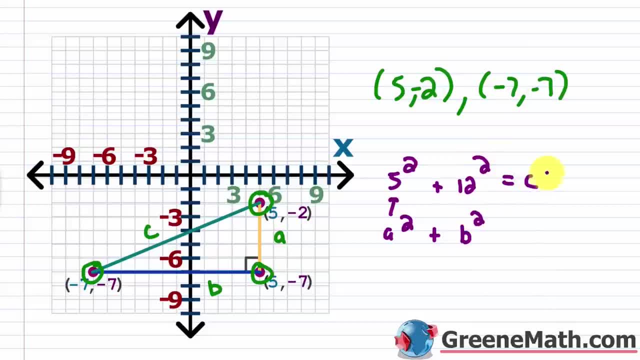 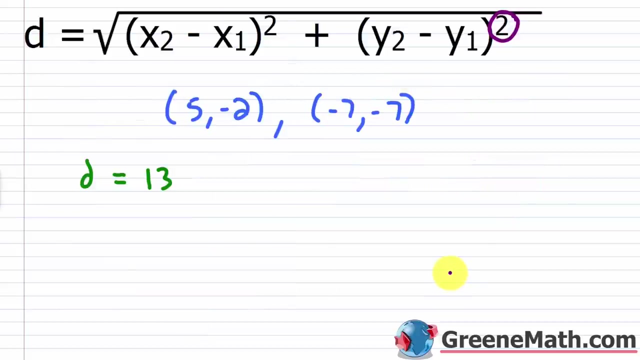 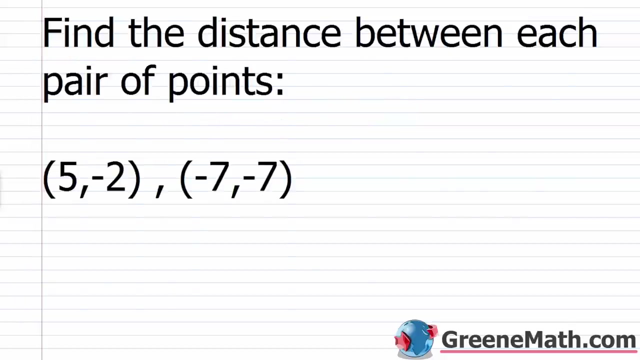 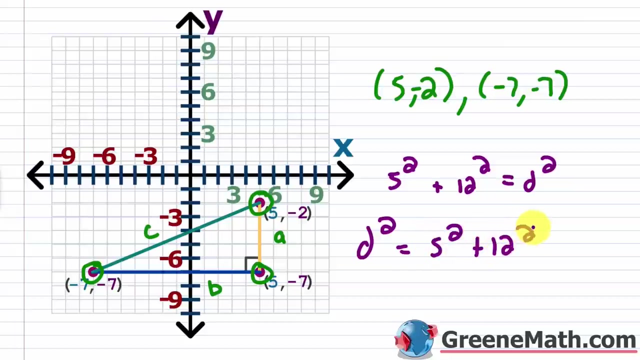 12. So we're squaring that. This is equal to C squared. Okay. C squared. And in this case, we just relabeled C with D for distance. That's all we did. So let's just label this as D. It doesn't matter. We're just changing the variables letter, but it means the same thing. Okay. So if I have D squared equals five squared plus 12 squared, how do I solve for D? Well, at this point, I can just take the square root of each side, right? I know I can simplify this further, but all I'm doing up here is I'm just taking the square root of each side. So I'm here. If I go back to my formula, once I have this guy, I can just take the square root of each side and I've solved for D. Okay. Let me go back down and make that crystal clear. So D squared equals, you have five squared plus 12 squared. If I take the square root of each side, then this would go away and I have the square root of this. Then I could just calculate this. Five squared is 25 and 12 squared is 144. And then 25 plus 144, is 169. And we all know the answer from earlier, D equals square root of 169, which is 13. Okay. 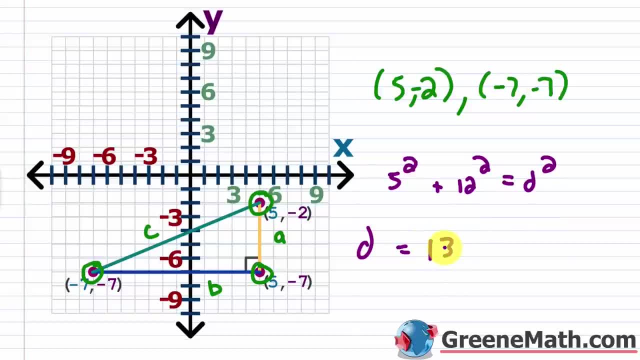 So just a quick insight into where this comes from. It's a direct application of the Pythagorean formula. I know most of you, you know, you're more interested in just being able to kind of get the formula and crank out your homework, but it's nice to know where it comes from. 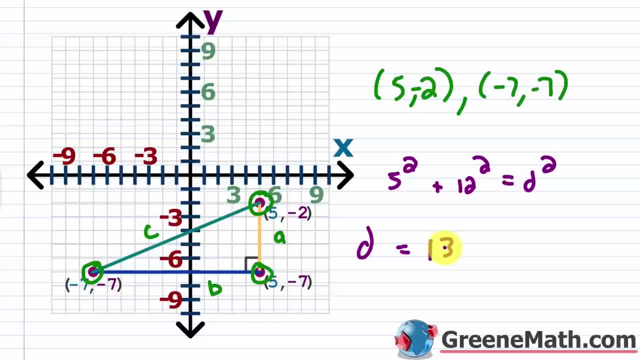 In case you forget the formula, you can kind of pull out a coordinate plane and kind of think your way through deriving this formula because it's very easy to get. You just need the difference in X value squared. And then you can kind of think your way through deriving this formula because it's very easy to get. You just need the difference in X value squared plus the difference in Y value 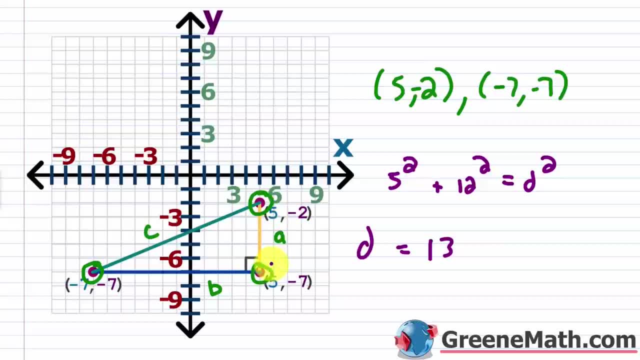 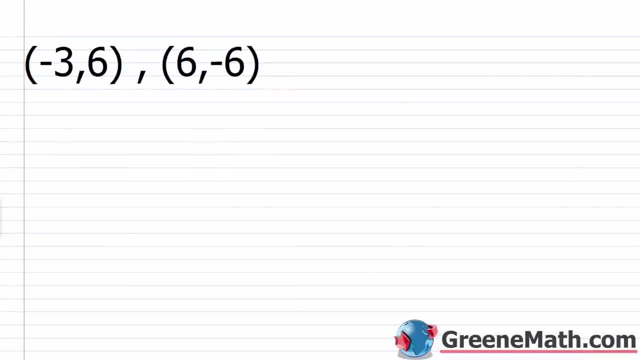 squared. That gives you your A squared plus B squared. Okay. And you set this equal to C squared. And from that, you can kind of set up your distance formula. All right. So now let's kind of wrap up the lesson by just kind of bursting through a few of these. Once you know, the formula is very, very easy. So we have that the distance between two points is equal to the 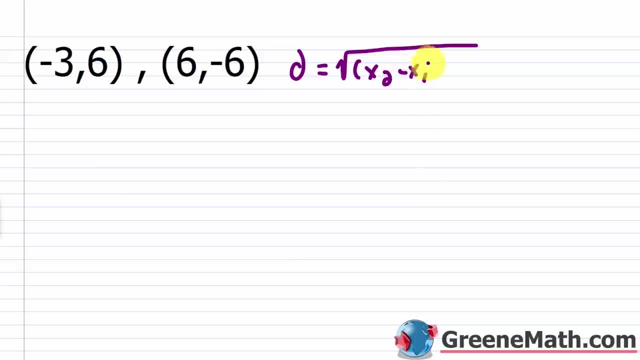 square root of, you've got X sub two minus X sub one quantity squared, plus you've got your Y sub two minus your Y. 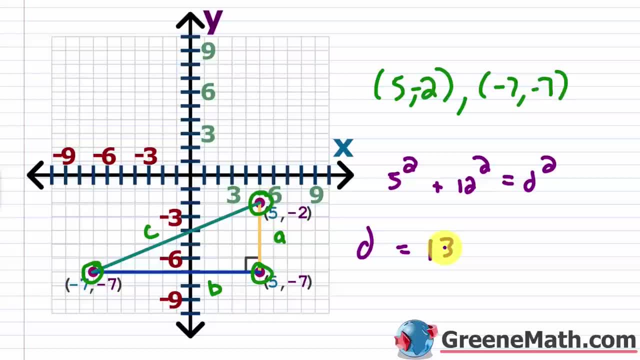 crank out your homework, but it's nice to know where it comes from, In case you forget the formula. you can kind of pull out a coordinate plane and kind of think your way through deriving this formula, because it's very easy to get. You just need the difference in X, value squared. 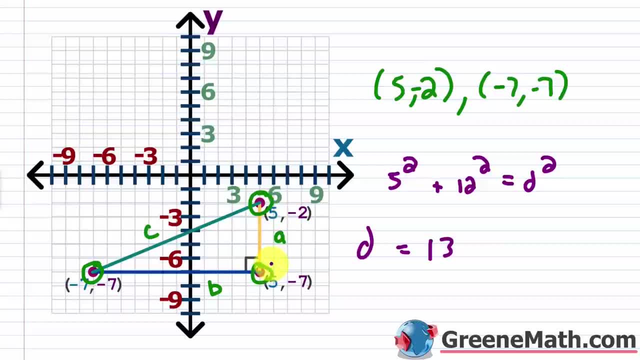 plus the difference in Y value squared, That gives you your A squared plus B squared, Okay, And you set this equal to C squared And from that you can kind of set up your distance formula. All right, So now let's kind of wrap up the lesson by just kind of bursting through a few of these. 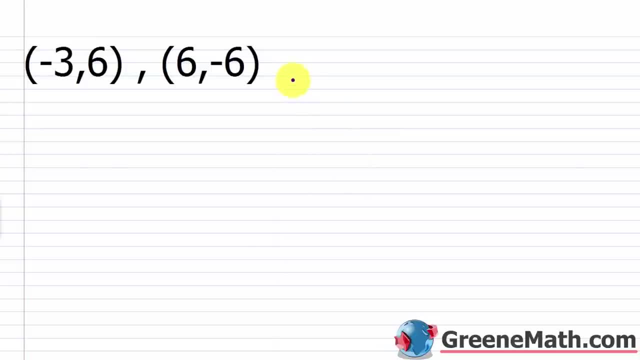 Once you know the formula you can kind of set up your distance formula. This formula is very, very easy. So we have that the distance between two points is equal to the square root of. you've got X sub two minus X sub one quantity squared plus. you've got your Y sub. 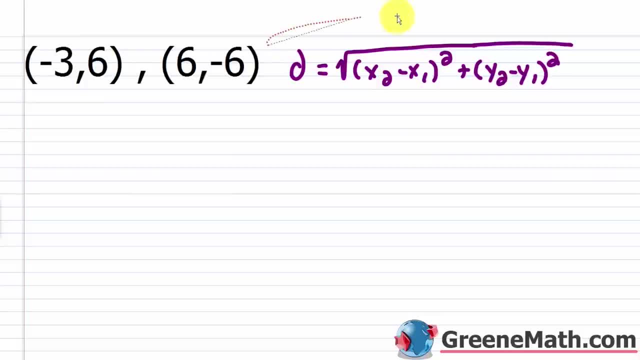 two minus your Y sub one, that quantity squared Okay, And I'll just drag this down here and let me put that right there. So this is going to be my X sub one, Y sub one. This is going to be my X sub two, Y sub two. Again, you can change that around, It doesn't matter. So just plug in real. 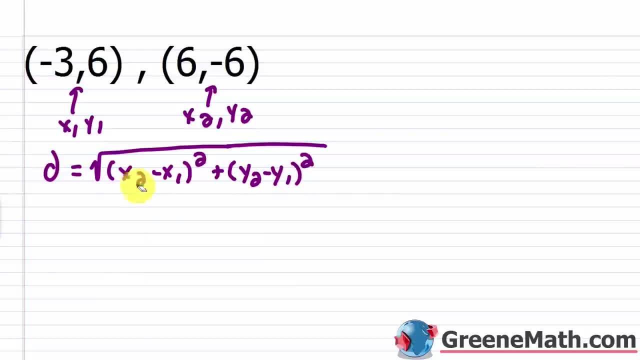 quick, We'll get our answer. So X sub two in this case is going to be six and X sub one is going to be negative three minus the negative three is plus three. Be very careful when you work with these. Whenever you have minus a. 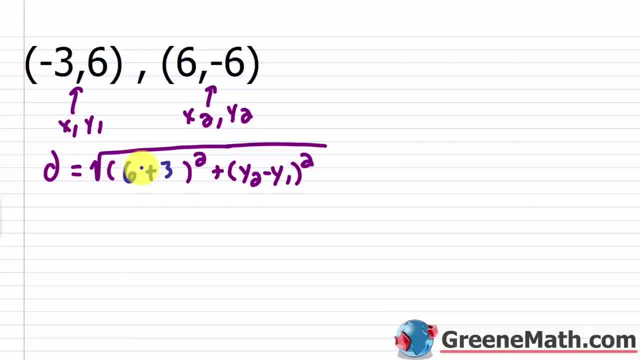 negative, you've got to make sure you do plus a positive. Okay, Very common mistake. So then Y sub two is going to be negative six and Y sub one is going to be positive six. So six plus three is nine. Nine squared is 81 and negative. six minus six is negative 12.. Negative: 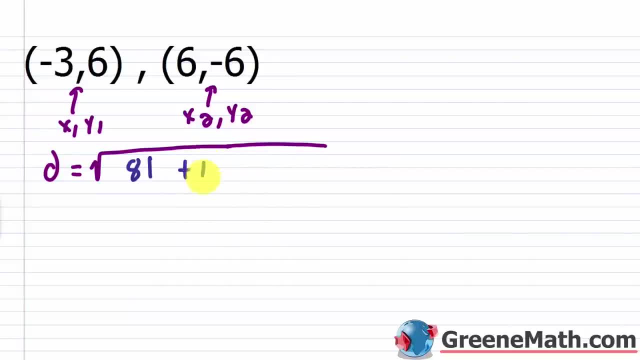 12 squared is 144.. So you get 81 plus 144, which is going to be 225.. And the principal squared of 225 is 15.. So the distance between these two points is going to be 15.. All right, let's take a look at. 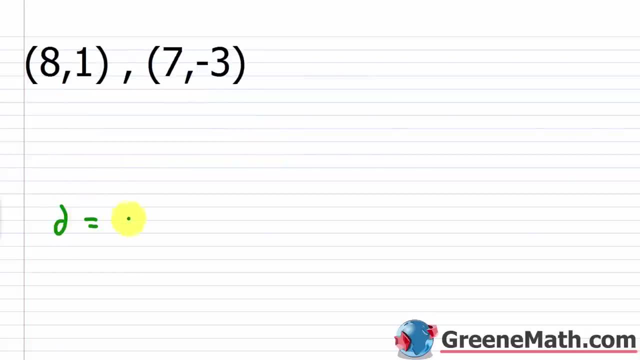 another one. So we have D. the distance between the two points is equal to the square root of. you've got your X sub two minus your X sub one- that quantity squared, plus your Y sub two minus your Y sub one- that quantity squared. And let me kind of make that a little bit more clear. 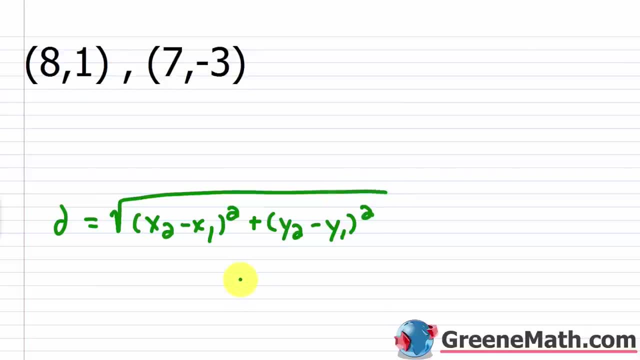 A little bit better. Okay, So let's just change it up and label this as X sub two, Y sub two. We'll label this as X sub one, Y sub one. Again, it does not matter how they're labeled, just like you saw. 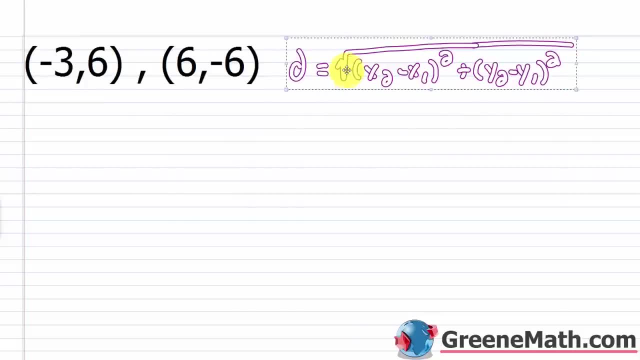 Sub one, that quantity squared. Okay. And I'll just drag this down here. And let me put that right there. So this is going to be my X sub one Y sub one. This is going to be my X sub two Y sub two. Again, you can change that around. It doesn't matter. So just plug in real quick. We'll get our answer. So X sub two in this case is going to be six and X sub one is going to be negative three minus the negative three is plus three. Be very careful when you work with these. Whenever you have minus a negative, you've got to make sure you do plus a positive. Okay. Very common mistake. So then Y sub two is going to be negative six and Y sub one is going to be positive six. So six plus three is nine, nine squared is 81. And negative six minus six is 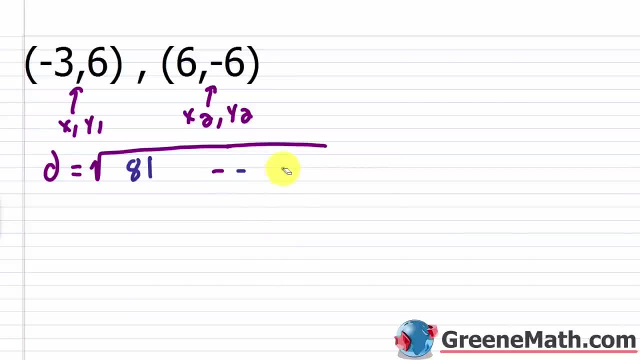 negative 12, negative 12 squared is 144. So you get 81 plus 144, which is going to be 225. 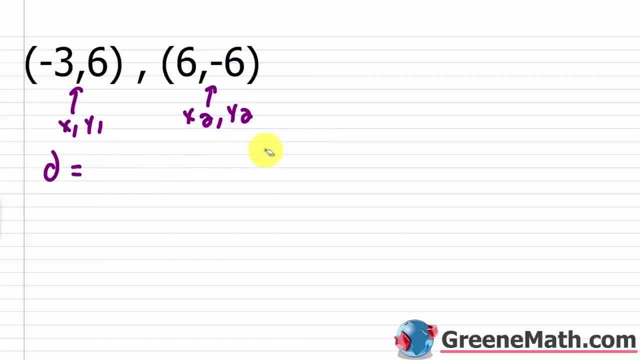 And the principal squared of 225 is 15. So the distance between these two points is going to be 15. All right. 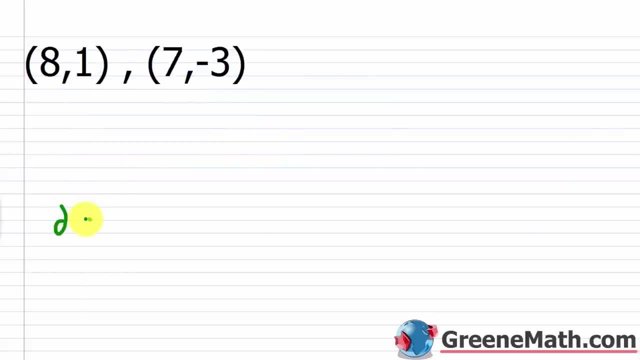 Let's take a look at another. So we have D, the distance between the two points is equal to the square root of, you've got your X sub two minus your X sub one, that quantity squared, plus your Y sub two minus your Y sub one, that quantity squared. And let me kind of make that a little bit better. Okay. So let's just change it up and label this as X sub two Y sub two. We'll label this as X sub one Y sub one. Again, it does not matter how they're labeled, just like you saw with slope formula. 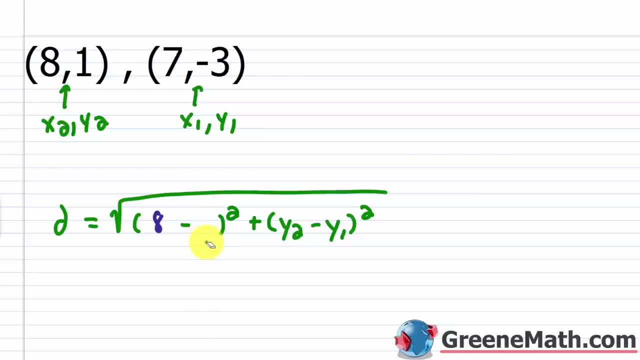 So for X sub two, I'm going to erase this and put eight. For X sub one, I'm going to erase this and put seven. You can go ahead and do that. Eight minus seven is one, one squared is one. Okay. So that's pretty simple. For Y sub two, I've got a one. For Y sub one, I've got a negative three. So again, be careful. Minus the negative three is plus three. And one plus three is obviously four. 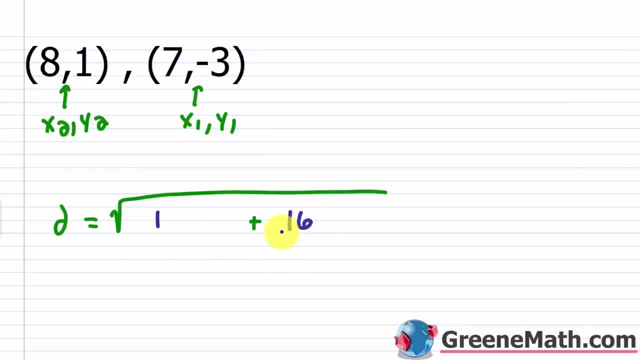 So if I have four squared, that gives me 16. One plus 16 is 17. So D, the distance equal to the square root of 17. Now, 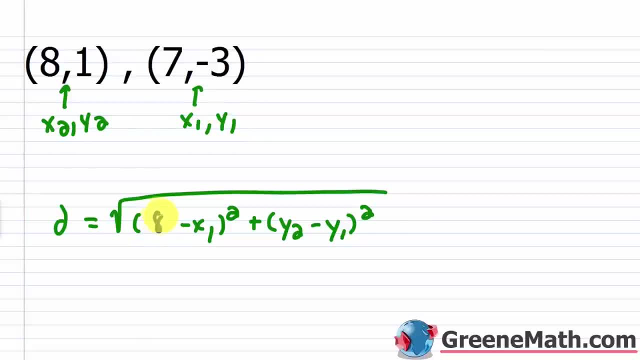 with slope formula. So for X sub two, I'm going to erase this and put eight. For X sub one, I'm going to erase this and put seven. You can go ahead and do that. Eight minus seven is one. one squared is one. Okay, So that's pretty simple. For Y sub two, I've got a one For Y sub one. 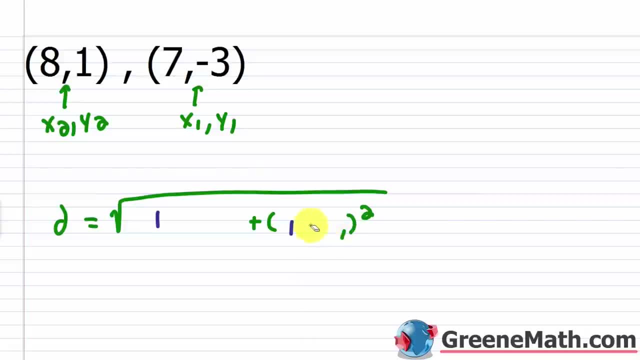 I've got a negative three, So again, be careful: Minus a negative three is plus three, And one plus three is obviously four. So if I have four squared, that gives me 16.. One plus 16 is 17.. So D, the distance equal to the square root of 17.. Now, 17 is not a perfect square. 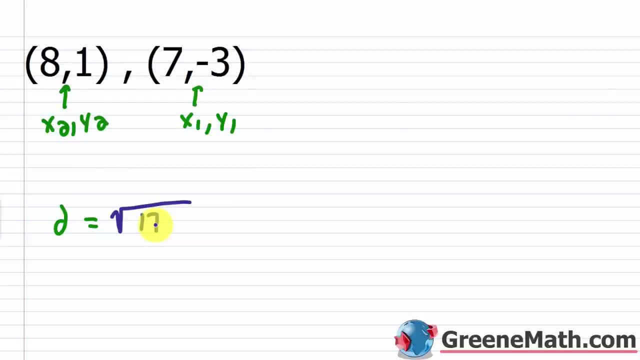 and 17 is a prime number, So it's not going to factor right, It's just one times 17.. So when you get an irrational number for your answer, then what you want to do is either leave it as the square root of 17, or you can approximate it. 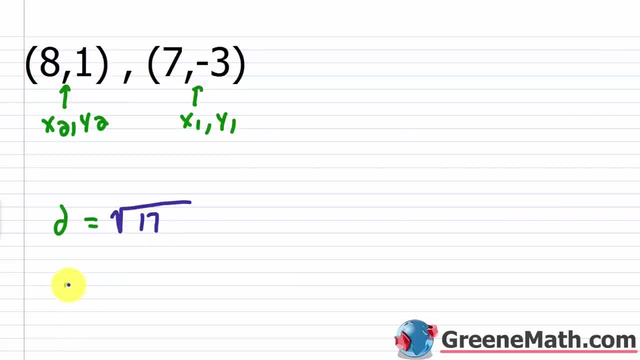 If you want to, but make sure you use the correct symbol, because it's not precise. So we could say: D is approximately 4.12.. Okay, It's approximately, or about 4.12.. Again, this is precise. D is equal. 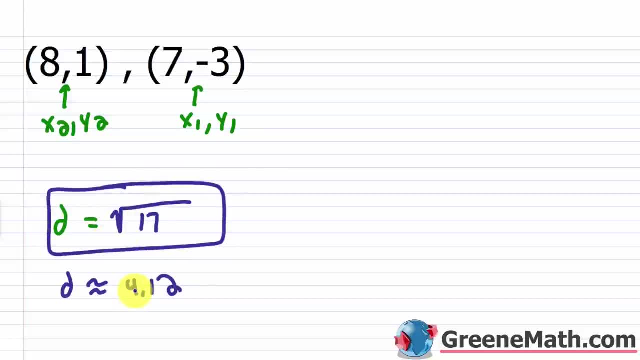 to the square root of 17.. I would always go with this answer, but sometimes it makes sense to do this, especially if you need to do some more calculations with it. All right, let's finish up the lesson and just look at one more. So we've got D. our distance between the two points is: 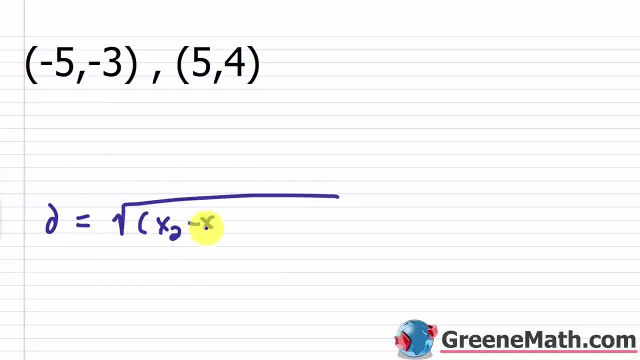 equal to the square root of again, you've got your X sub two minus your X sub one squared. Let me make that a little better, a little clearer. Plus, you've got your Y sub two minus your Y sub one squared, And let me make that a little better, Okay. 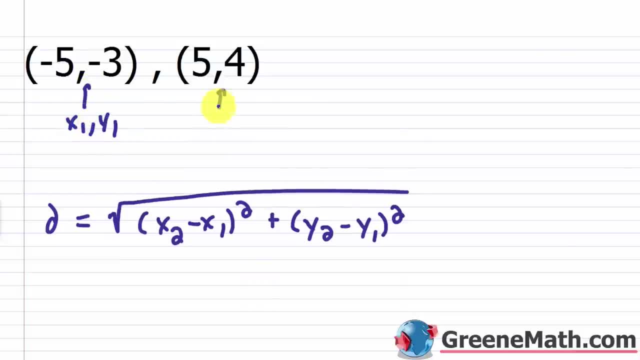 So I'll label this as X sub one, Y sub one, and this is X sub two, Y sub two, And again we're just going to plug in. So for X sub two, I'm going to plug in a five For X sub one. 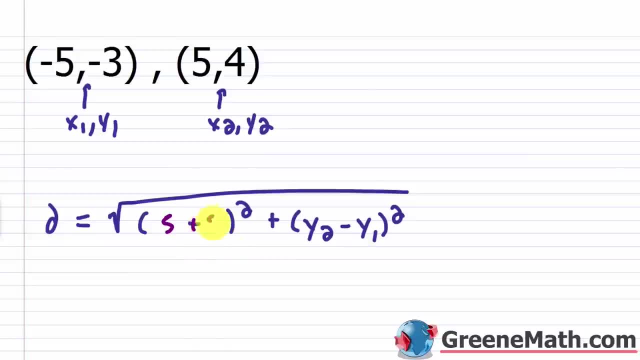 I'm going to plug in a negative five. So minus a negative five is plus five. So five plus five is 10, 10 squared is a hundred. Okay, So this is a hundred. So I'm going to plug in a negative five. 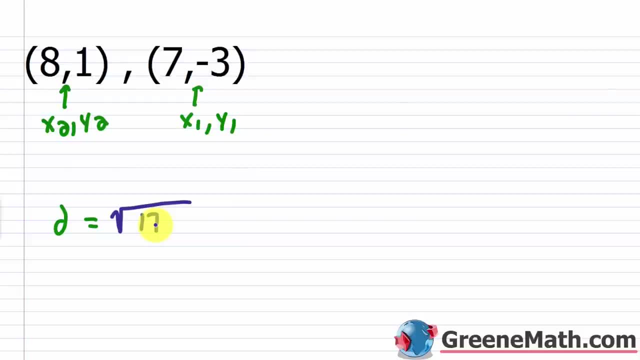 17 is not a perfect square, and 17 is a prime number. So it's not going to factor, right? It's just one times 17. So when you get an irrational number for your answer, then what you want to do is either leave it as the square root of 17, or you can approximate it if you want to. But make sure you use the correct symbol because it's not precise. So we could say D is approximately 4.12. Okay. It's approximately or about 4.12. Again, this is precise. D is equal to the square root of 17. I would always go with this answer, but sometimes it makes sense to do this, especially if you need to do some more calculations with it. 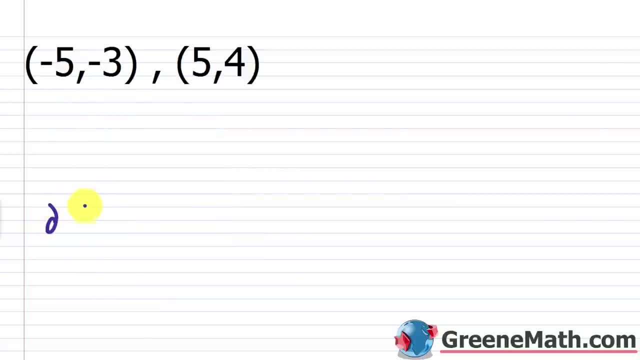 All right. Let's finish up the lesson and just look at one more. So we've got D, our distance between the two points, is equal to the square root of, again, you've got your X sub two minus your X sub one squared. Let me make that a little better, a little clearer. Plus, you've got your Y sub two minus your Y sub one squared. And let me make that a little better. Okay. So I'll label this as X sub one, Y sub one. And this is X sub two, Y sub two. And again, we're just going to plug in. So for X sub two, I'm going to plug in a five. For X sub one, I'm going to plug in a negative five. So minus a negative five is plus five. So five plus five is 10. 10 squared is 100. Okay. So this is 100. And then Y sub two is going to be four. And Y sub one is negative three. Again, minus a negative three is plus three. So four plus three is going to be seven. 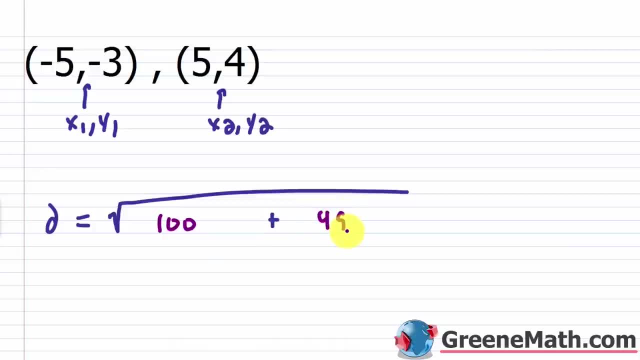 Square root is 49. Okay. So now you've got 100 plus 49, which is 149. Okay, 149. And again, 149 is a prime number. So I'm just going to leave my answer like this. I'm just going to say D is equal to the square root of 149. Just like that. If you want to approximate it, you can, you can say D, the distance is approximately going to be 12.21. Okay, just as an approximation. But this guy right here is a precise answer. Whereas this one, 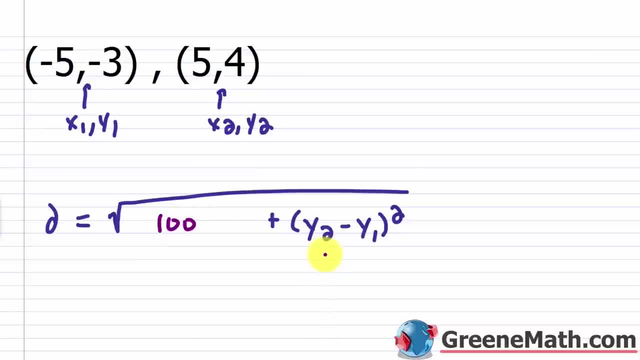 A hundred, And then Y sub two is going to be four, And Y sub one is negative three. Again, minus a negative three is plus three. So four plus three is going to be seven. Seven squared is 49.. Okay, So now you've got a hundred plus 49,, which is 149.. Okay, 149.. And again, 149 is a prime. 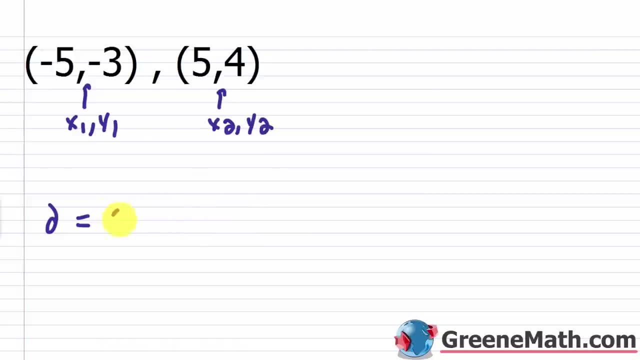 number. So I'm just going to leave my answer like this. I'm just going to say D is equal to the square root of 149, just like that. If you want to approximate it, you can. you can say D: the distance is approximately going to be. 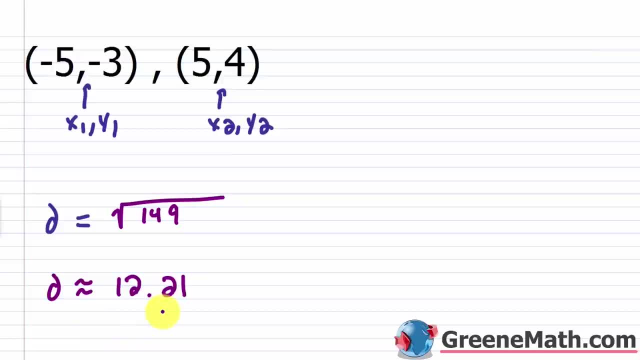 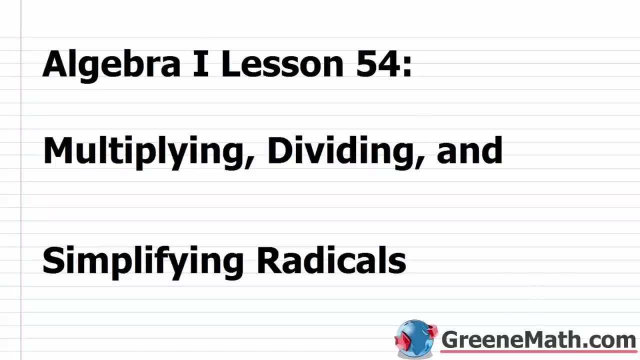 12.21.. Okay, Just as an approximation, but this guy right here is a precise answer, Whereas this one is just an estimate. Hello and welcome to Algebra 1, Lesson 54.. In this video, we're going to learn about multiplying, dividing and simplifying radicals. All right, So let's. 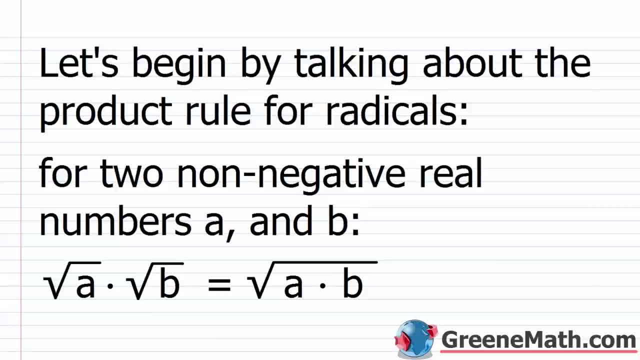 begin today by talking about the product rule for radicals. So this is the very, very first thing that's going to be in your textbook when you start talking about simplifying radicals. So let me highlight that Again: the product rule for radicals. So you're going to 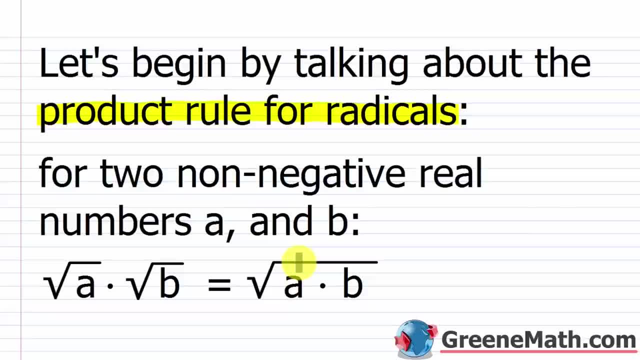 see something similar again in your textbook And it's going to start out by just saying that for two non-negative real numbers, let's just say A and B, and they could be any two letters you want to use. We have that the square root of A times the square root of B is equal to the square root. 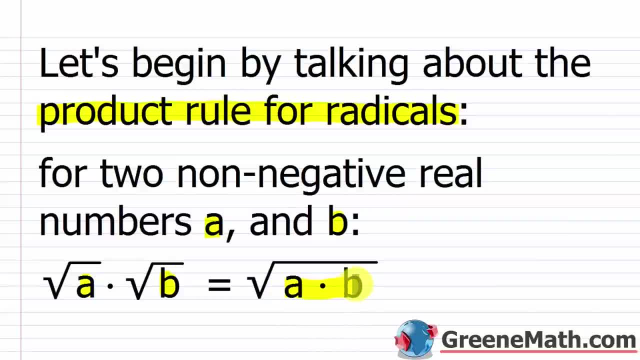 of A times B. Now, a lot of times when we see these kind of abstract concepts in our textbook, it's hard to relate them to the problems we're going to see on our homework or on a test or you know wherever we might see them. But it's very easy to kind of 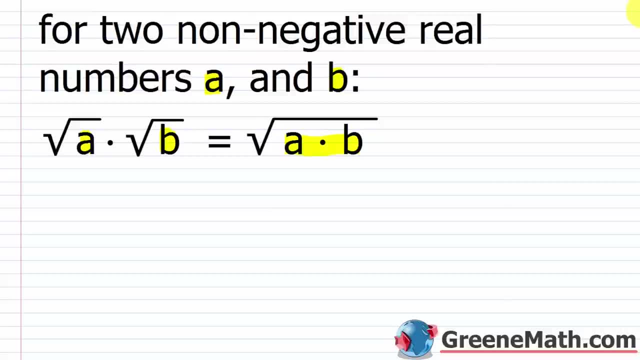 just work with things we already know and prove these concepts. So if I had something like the square root of 4, and I multiply this by the square root of 9. Now we should be able to look at this rule and just kind of match this up and say, okay, well, based on this rule, 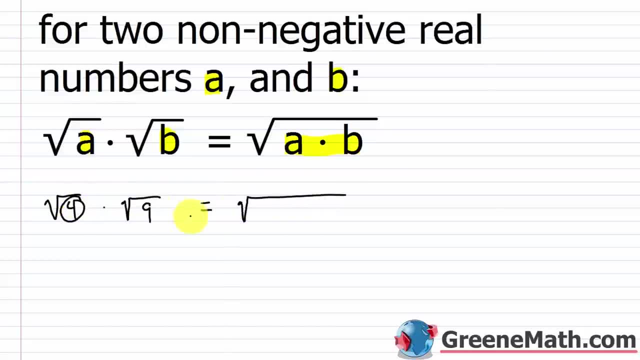 we're going to be able to do the square root of 4 times 9.. So the square root of 4 times 9, which would be equal to what The square root of 4 times 9, is 36.. And we know 36 is a perfect. 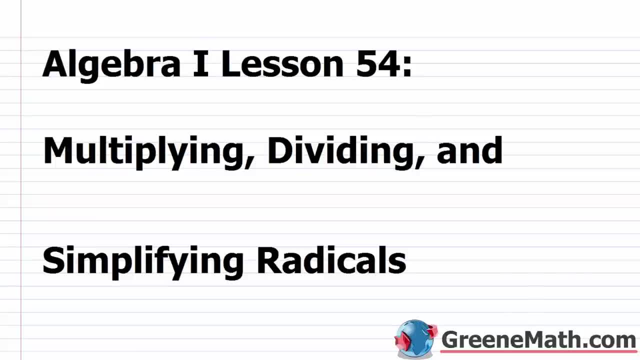 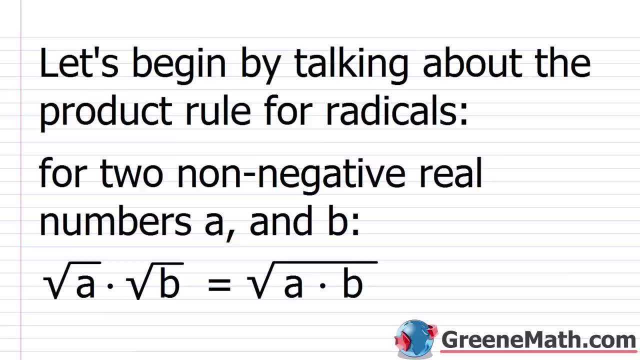 is just an estimate. Hello, and welcome to Algebra One Lesson 54. In this video, we're going to learn about multiplying, dividing and simplifying radicals. All right, so let's begin today by talking about the product rule for radicals. So this is the very first thing that's going to be in your textbook, when you start talking about simplifying radicals. So let me highlight that. Again, the product rule for radicals. So you're going to see something similar again in your textbook. And it's going to start out by just saying, that for two non-negative real numbers, let's just say A and B, and they could be any two letters you want to use, we have that the square root of A times the square root of B is equal to the square root of A times B. Now, a lot of times when we see these kind of abstract concepts in our textbook, it's hard to relate them to the problems we're going to see on our homework, 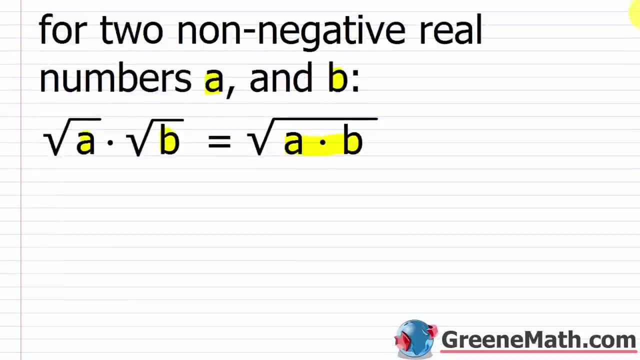 or on a test or, you know, wherever we might see them. But it's very easy to kind of just work with things we already know. So let's get started. So the first thing that we're going to do is we're 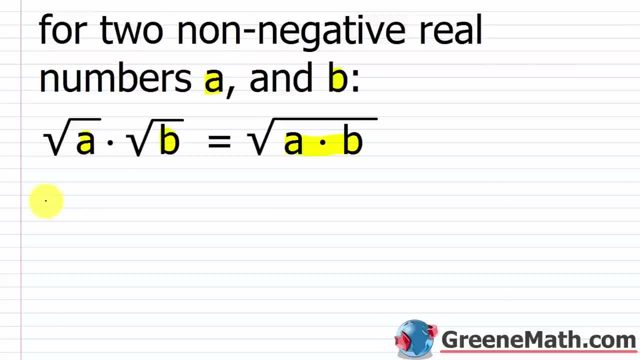 going to have to do is we're going to have to do a little math. So if I had something like the square root of four, and I multiply this by the square root of nine. Now, we should be able to look at this rule and just kind of match this up and say, okay, well, based on this rule, I should be able to do the square root of four times nine. So the square root of four times nine, 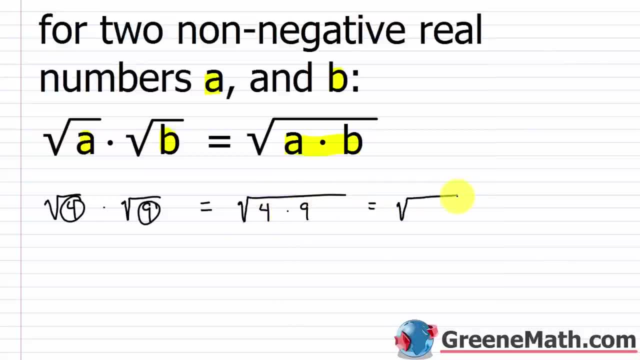 which would be equal to what the square root of four times nine is 36. And we know 36 is a perfect square, right? It's six times six. So the answer here would just be six. Now, can we prove that this is mathematically valid? Yes, we can. We know that the square root 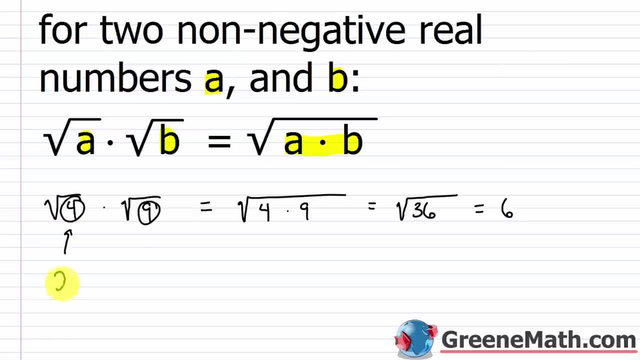 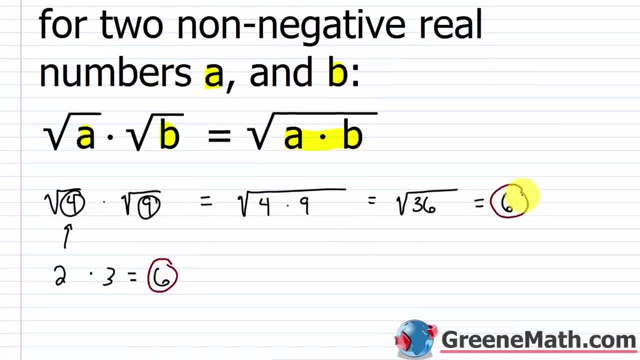 of four is two. So I could basically write that this is two times the square root of nine, we know that's three. So two times three is what? It's six. So the end result here is the same, I got six this way. And I got six this way. Right? Now, I could also have reversed that I could have 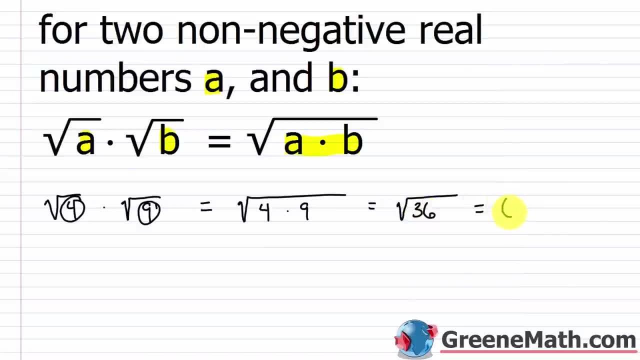 square right It's 6 times 6.. So the answer here would just be 6.. Now can we prove that this is mathematically valid? Yes, we can. We know that the square root of 4 is 2.. So I could basically: 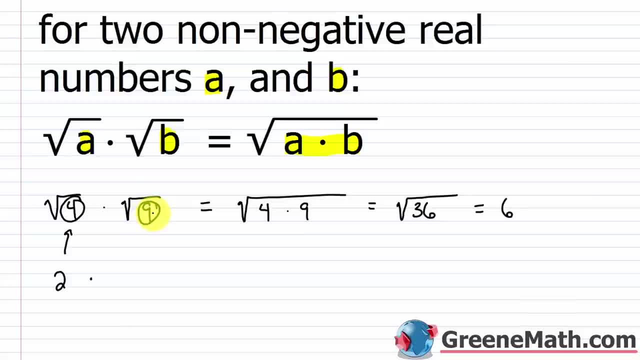 write that this is 2 times 9.. And we know that the square root of 4 is 2.. So I could basically write that this is 2 times the square root of 9.. We know that's 3.. So 2 times 3 is what It's 6.. 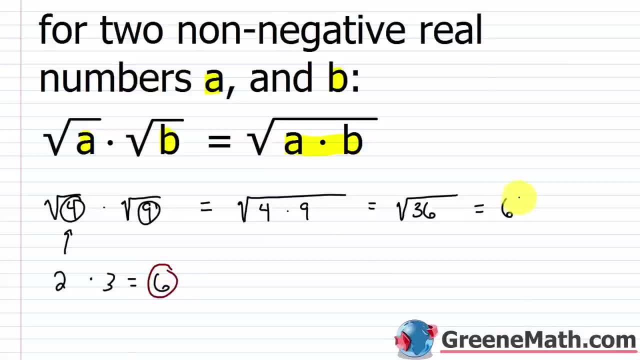 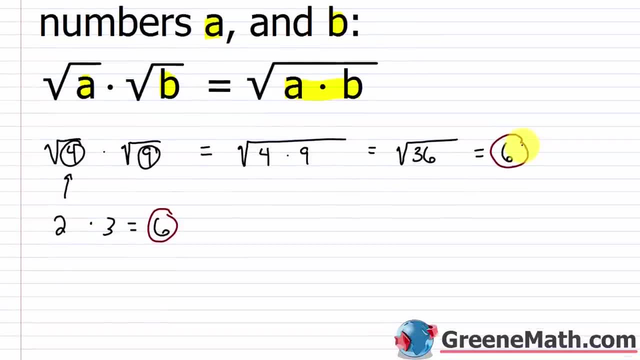 So the end result here is the same. I got 6 this way and I got 6 this way right Now. I could also have reversed that. I could have started out with something like the square root of 36. And I could have factored it. I could have factored into the square root of 4 times 9.. And 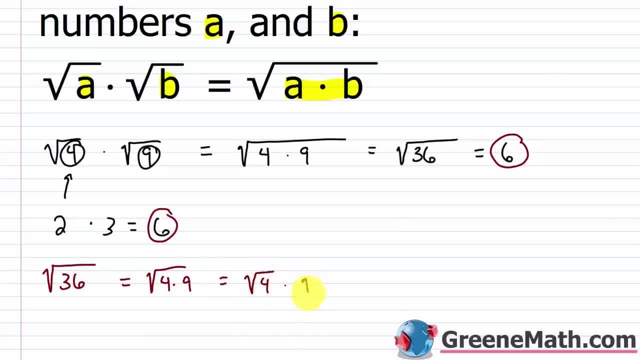 then I could have broke it up and say, okay, this is the square root of 4 times the square root of 9.. I could have said: okay, well, the square root of 4 times 9 is 36.. And then I could have: 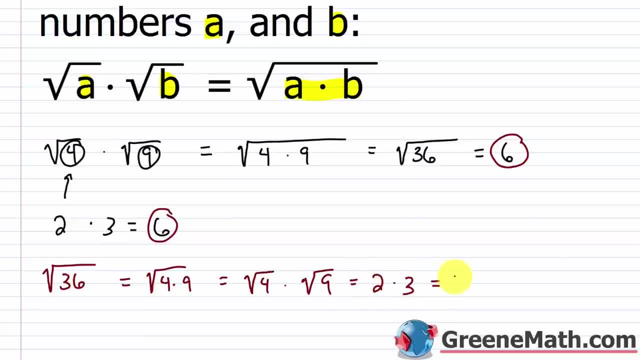 said: okay, well, the square root of 4 is 2 times the square root of 9, which is 3.. And I could have got 6 that way. So you're allowed to go back and forth. So let's look at another, just quick. 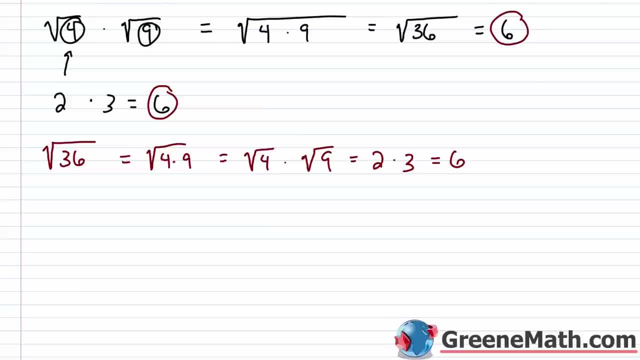 kind of example. Let's take two square roots that we know already. We know that the square root of 16 is 4.. So let's do the square root of 16.. And let's multiply this by the square root of 25,. 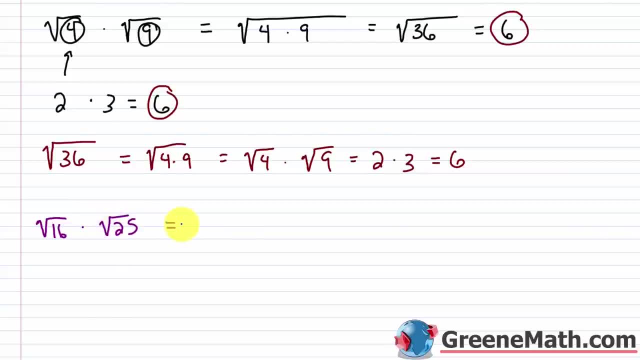 right, We know that's 5.. So by this rule again, I can do this as the square root of 16 times 25.. And 16 times 25 is 400.. So this equals the square root of 400. And we should. 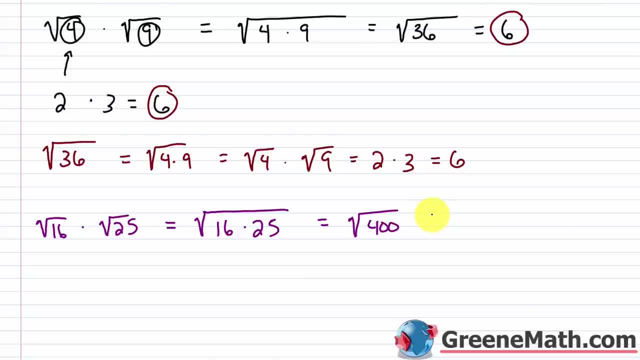 know from the videos we've done so far that the square root of 400 is 20, right, So this would be 20.. Now again, there's multiple ways to kind of look at this. I could have started out with the square root of 400. And I could have said: well, I don't know what that is, So let me break. 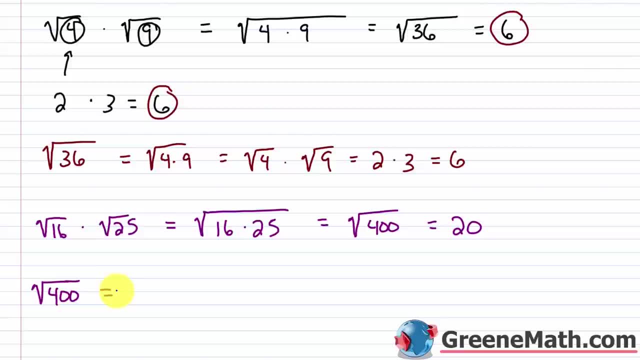 that down. I could use a factor tree and I could find out that 16 and 25 are factors of 400.. So I could say: okay, I can break this down into the square root of 16 times the square root of 25.. And then these are two square roots that I know, right, Square root. 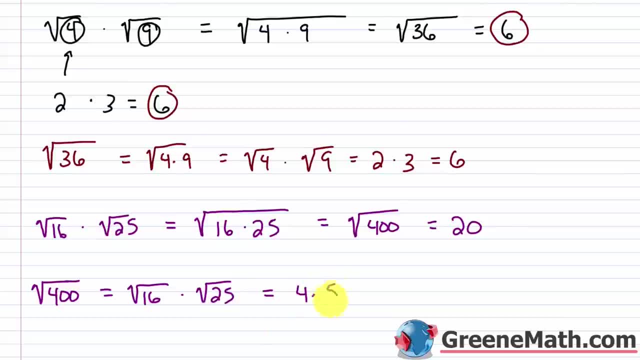 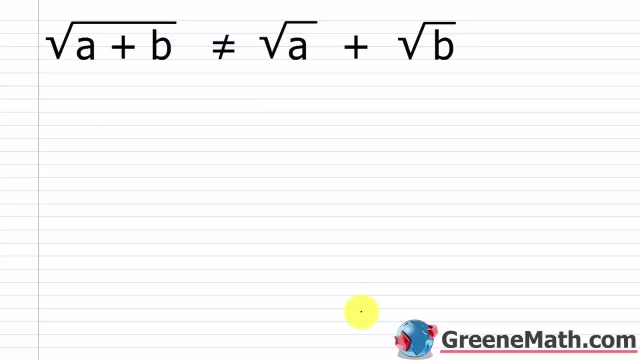 of 16 is 4 times square root of 25 is 5.. 4 times 5, I know, is 20.. So again, another way to kind of get that answer. All right, So before we kind of move on, I want to address something that comes. 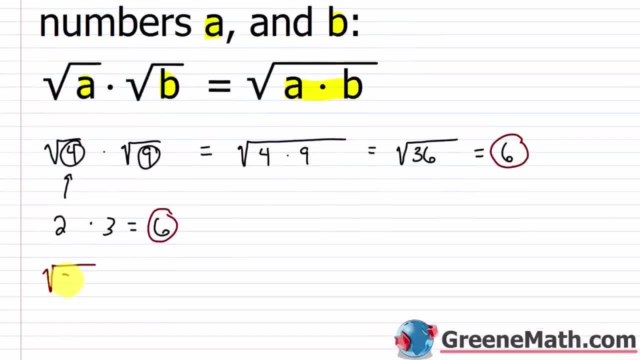 with something like the square root of 36. And I could have factored it, I could have factored into the square root of four times nine. And then I could have broke it up and say, okay, this is the square root of four times the square root of nine, I could have said, okay, well, the square root of 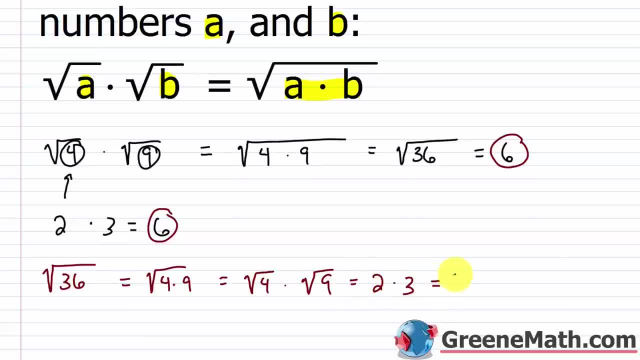 four is two times the square root of nine, which is three, and I could have got six that way. 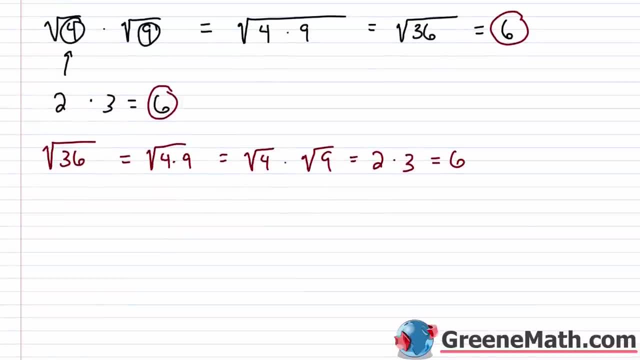 So you're allowed to go back and forth. So let's look at another just quick kind of example. 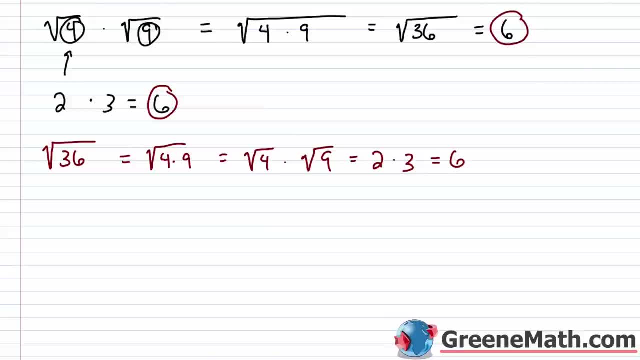 Let's take two square roots that we know already. The square root of 16 is four. So let's do the square root of 16. 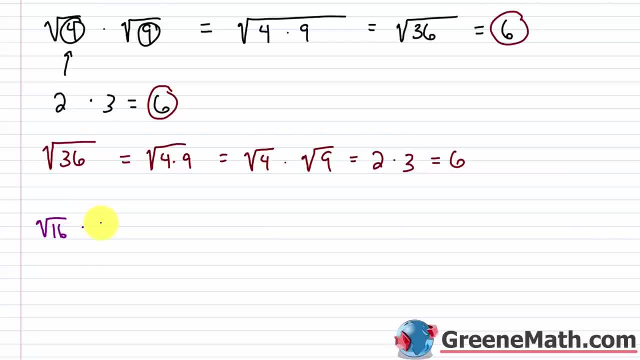 And let's multiply this by the square root of 25. Right? We know that's five. 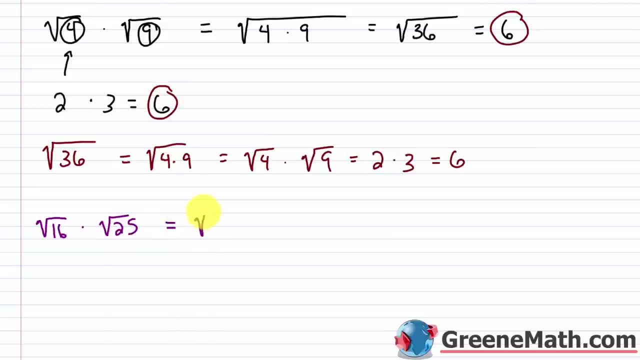 So by this rule, again, I can do this as the square root of 16 times 25. And 16 times 25 is 400. So this equals the square root of 400. And we should know from the videos we've done so far, that the square root of 400 is 20. Right? So this would be the square root of 25. And we should know from the videos we've done so far, that this would be 20. Now, again, there's multiple ways to kind of look at this, I could have started out with the square root of 400. And I could have said, well, I don't know what that is. So let me break that down. I could use a factor tree. And I could find out that 16 and 25 are factors of 400. So I could say, okay, I can break this down into the square root of 16 times the square root of 25. And then these are two square roots that I know, right square root of 16 is four times square root of 25 is five. 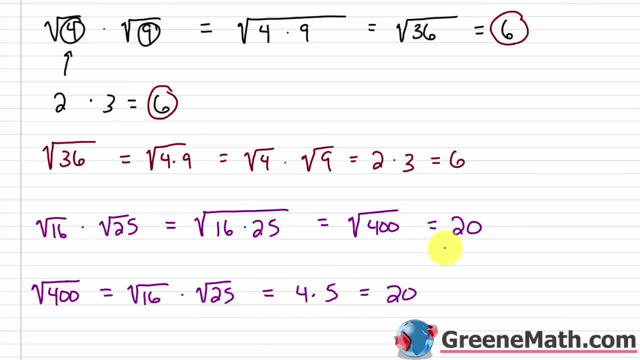 Four times five, I know is 20. So again, another way to kind of get that answer. All right. So 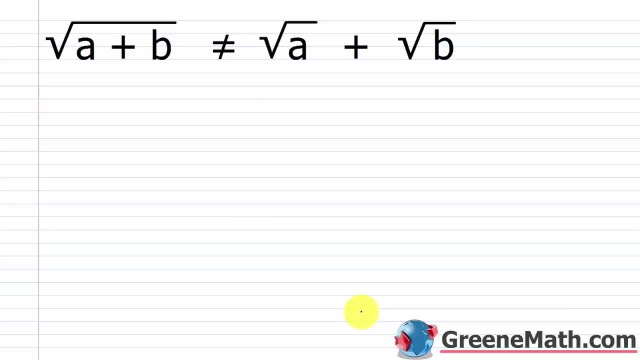 before we kind of move on, I want to address something that comes up pretty often. It's a very, very common mistake that you're going to see. So in general, if you have the square root of a plus b, okay, notice how there's an addition sign there. This is addition. This is generally not equal to the square root of a plus the square root of b. And there are some exceptions to this. If I did the square root of zero plus one, this would be equal to the square root of zero plus the square root of one, right? This is going to be equal to one. And so is this, right? So in some circumstances, you can make it work. But when we have a rule, okay, that we're going to follow, it's got to work for everything. It's got to be completely consistent. I got to be able to rely on it. And I can't rely on this because this isn't going to work in the majority of cases. Okay, let me give you a quick example. Let's say you had something like the square root of four plus four. This would be what? If I simplified this correctly, I would just perform the operation under the square root symbol. So I would do four plus four is eight. So this is the square root of eight. And if I approximated this, because this is an irrational number, I would get about 2.83, let's say. And that's an estimate. It's not an exact value, but it's close enough, 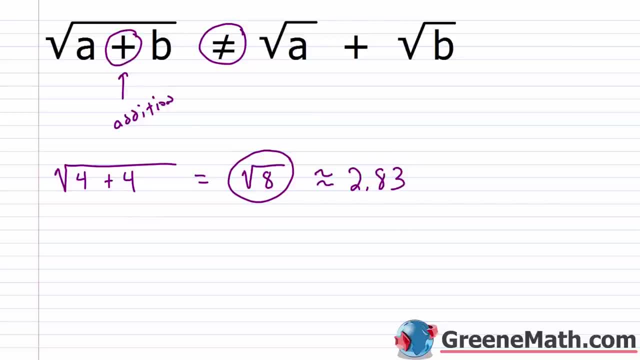 to prove our point here. If I was able to simplify the way that most students think that I can, I could go, okay, this is the square root of four plus four. And I'll just separate this. So this is the square root of four plus the square root of four. Well, I know the square root of four is two. So this would be what? It would be two plus two. So this should equal four if this logic was correct, but it's not, right? Because this is the square root of eight and it's about 2.83. So that's why this is, 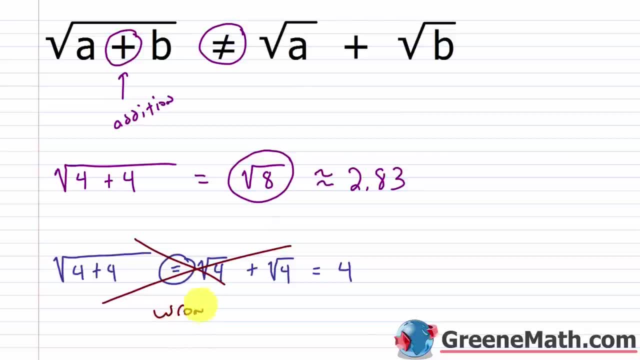 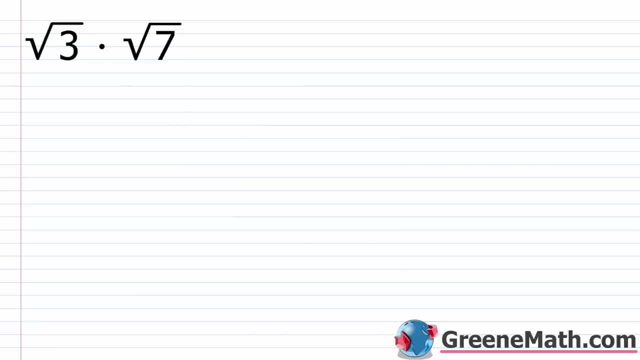 let me put some big red through this. This is wrong. Okay. This is incorrect. And again, a lot of students make that mistake. Please don't be one of them. All right. So let's use the product rule for radicals to do some basic multiplication here. You'll see some problems like this at the beginning of the section. So you have something like the square root of three times the square root of seven. What I can do is write this as the square root of three times seven. 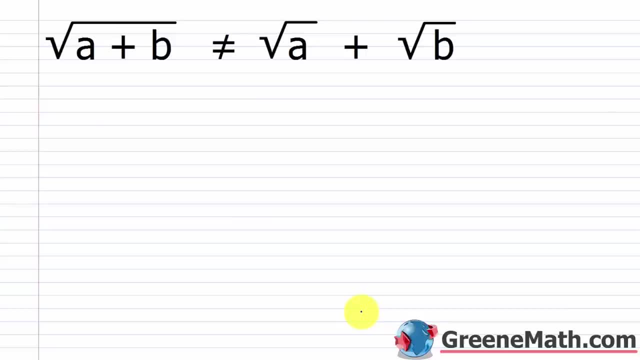 up pretty often. It's a very, very common mistake that you're going to see. So, in general, if you have the square root of a plus b, which is the square root of a plus b, which is the square root of b, Okay, Notice how there's an addition sign there. This is addition. This is generally not. 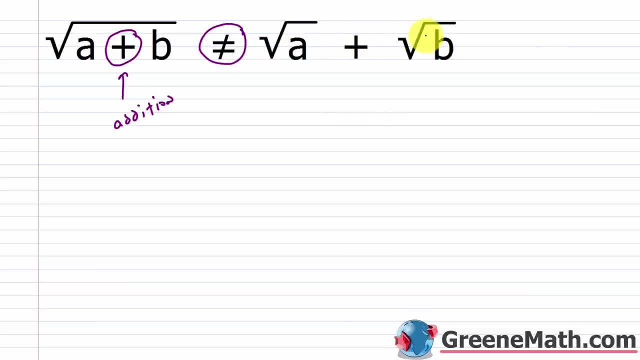 equal to the square root of a plus the square root of b, And there are some exceptions to this. If I did the square root of 0 plus 1, this would be equal to the square root of 0 plus the square root of 1, right? This is going to be equal to 1, and so is this right. So in some circumstances, 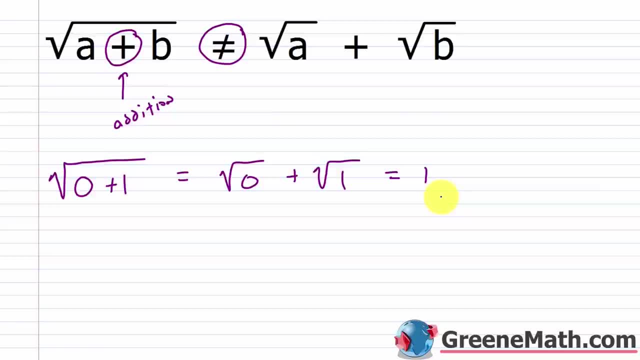 you can make it work, But when we have a rule, okay, that we're going to follow, it's got to work for everything. It's got to be completely consistent. I got to be able to rely on it, And I can't rely on this because this isn't going to. 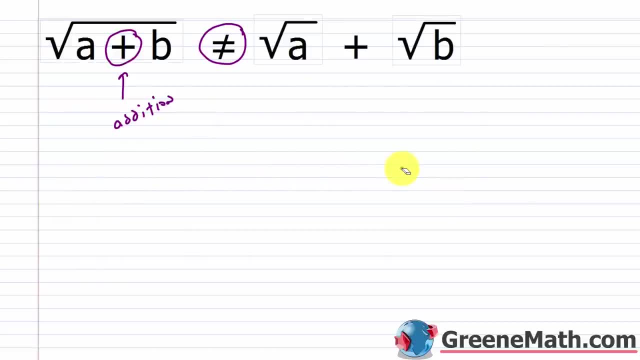 work in the majority of cases. Okay, If I want to give you a quick example, let's say you had something like the square root of 4 plus 4.. This would be what If I simplified this correctly? I would just perform the operation under the square root symbol. So I would do 4 plus 4 is. 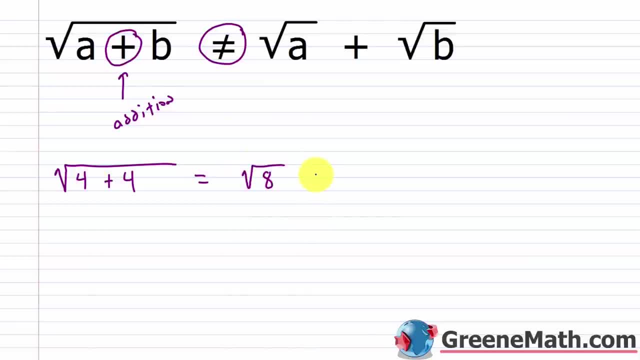 8.. So this is the square root of 8.. And I would do: 4 plus 4 is 8.. So this is the square root of 8.. And if I approximated this, because this is an irrational number, I would get about 2.83,. 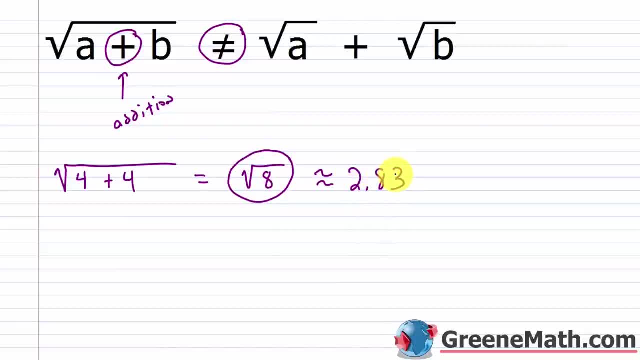 let's say, And that's an estimate, It's not an exact value, but it's close enough to prove our point here. If I was able to simplify the way that most students think that I can, I could go: okay, this is the square root of 4 plus 4.. And I'll just separate this. So this is the square. 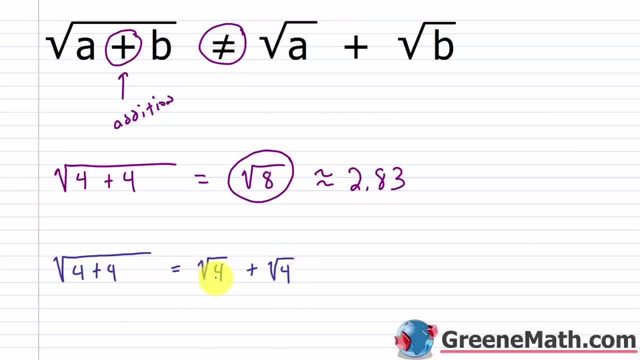 root of 4 plus the square root of 4.. Well, I know, the square root of 4 is 2.. So this would be what It would be: 2 plus 2.. So this should equal 4 if this logic was correct. 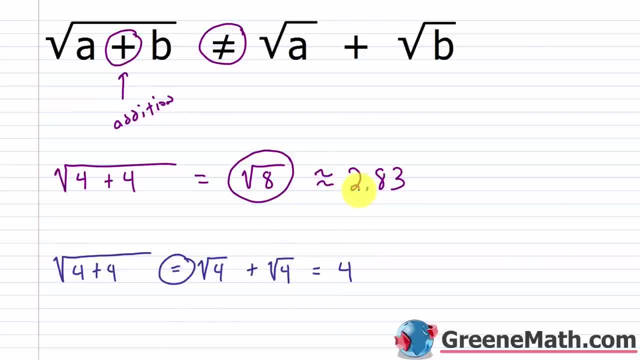 but it's not right, Because this is the square root of 8, and it's about 2.83.. So that's why this is. let me put some big red through this. This is wrong. Okay, This is incorrect, And again. 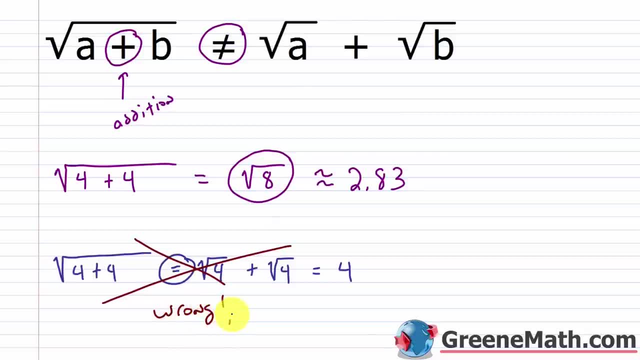 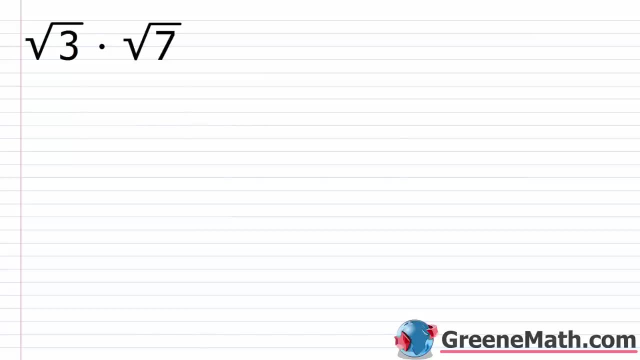 a lot of students make that mistake. Please don't be one of them. All right, So let's use the product rule for radicals to do some basic multiplication here. You'll see some problems like this at the beginning of the section. So you have something like the square root of 3 times the square root. 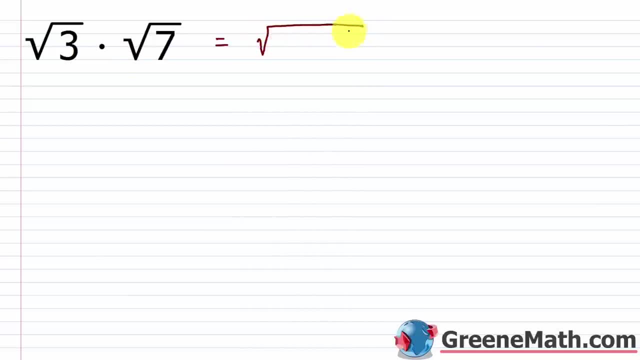 of 7.. What I can do is write this as the square root of 3 times 7.. So 3 times 7.. So this is equal to the square root of 21.. So just a way to combine things that make it simpler. Here's another one. 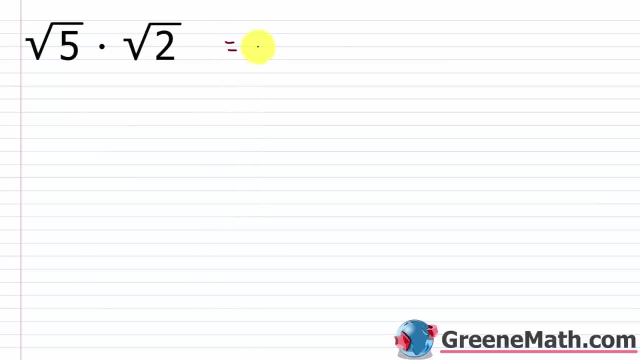 We have the square root of 5 times the square root of 2.. So I can say this is equal to the square root of 5 times 2.. 5 times 2 is equal to the square root of 10.. What about the square root? 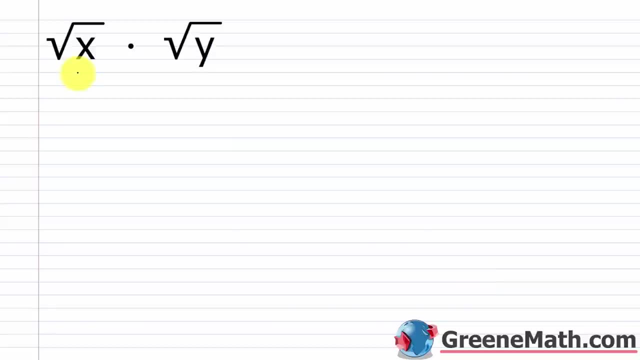 of x times the square root of y. Well, even though there are variables involved, we're still going to follow the same process, So I can write this as the square root of x times y, x times y, or just the square root of xy. Remember, variables represent numbers, So the properties that we use. 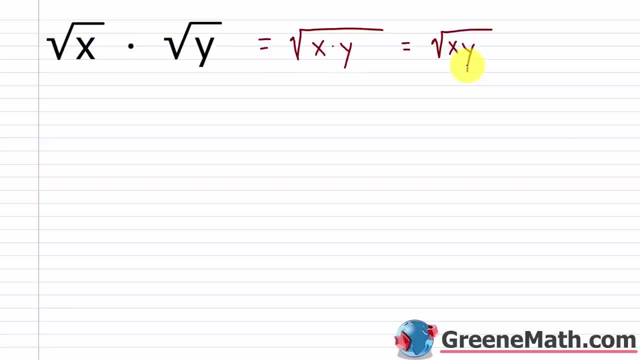 with numbers we use with variables, right, Because they're just representing those numbers. We just don't know what they are. What about the square root of 13x times the square root of 11y? Again, just equals the square root of: I'll have 13 times 11 times x times y, So this equals. 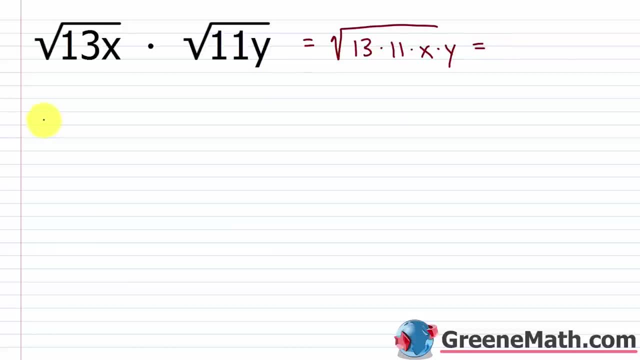 13 times 11 is 143. So this would be the square root of 143, xy xy. So even if you had more than two of these, you still follow the same process. So I've had the square root of 2 times the square. 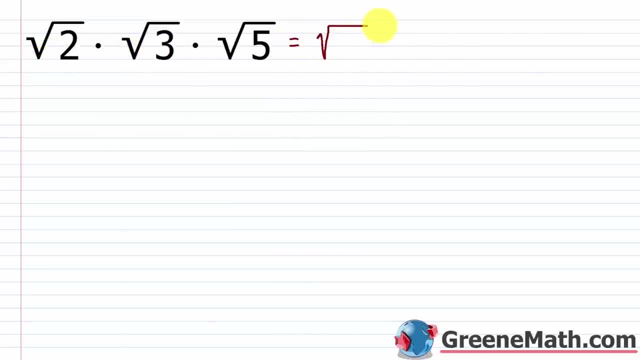 root of 3 times the square root of 5.. I can write this as: the square root of 2 times 3 times 5.. So 2 times 3 times 5.. So this is equal to: we'll have the square root of. 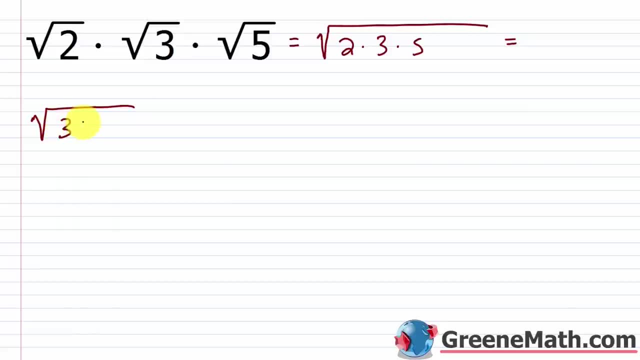 2 times 3 is 6,, 6 times 5 is 30. So the square root of 30. So pretty easy overall to use the product rule for radicals. That's kind of the first type of problem you're going to encounter. 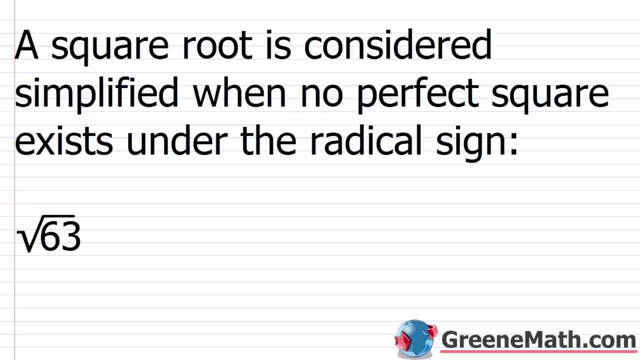 in this section. Then you're going to kind of move on and talk about simplifying radicals. So this is where you've got to take this rule that you just learned and kind of apply it. So a square root is considered a square root of x. So this is where you've got to take this rule that you just 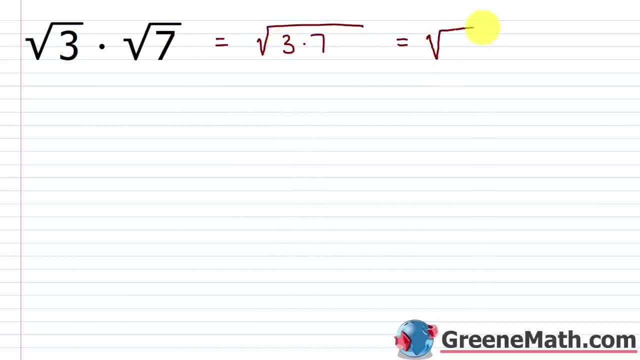 So three times seven. So this is equal to the square root of 21. 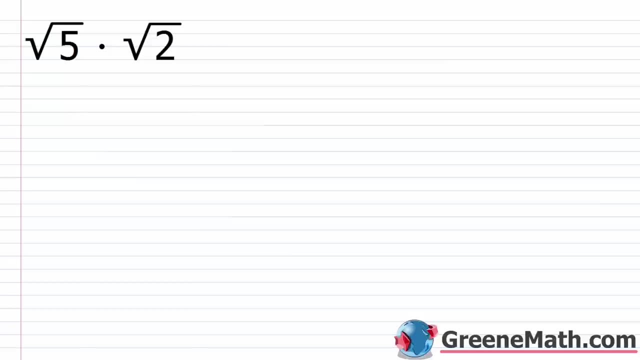 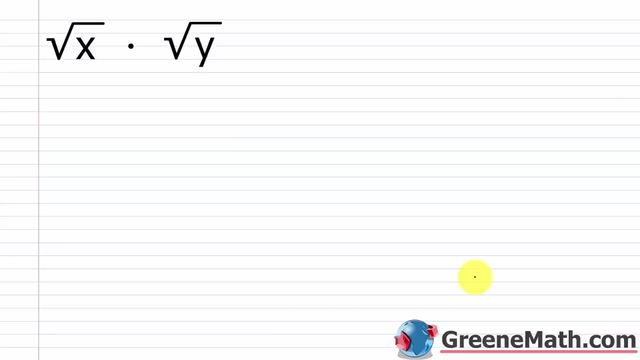 So just a way to combine things that make it simpler. Here's another one. We have the square root of five times the square root of two. So I can say this is equal to the square root of five times two, five times two is equal to the square root of 10. What about the square root of X times the square root of Y? Well, even though there are variables involved, we're still going to follow the same process. So I can write this as the square root of X times Y, X times Y, or just the square root of X, Y. Remember, variables represent numbers. So the properties that we use with numbers, we use with variables, right? Because they're just representing those numbers. We just don't know what they are. What about the square root of 13X times the square root of 11Y? Again, just equals the square root of, I'll have 13 times 11 times X times Y. 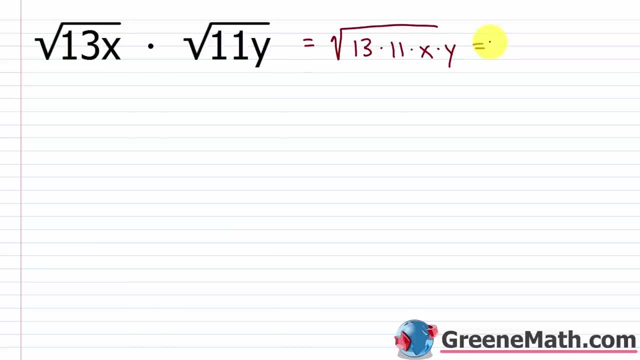 So this equals 13 times 11 is 143. So this would be the square root of X times Y. So even if you had more than two of these, you still follow the same process. So I've had the square root of two times the square root of three times the square root of five. I can write this as the square root of two times three times five. So two times three times five. So this is equal to, we'll have the square root of two times three is six, six times five is 30. So the square root of 30. So pretty easy. 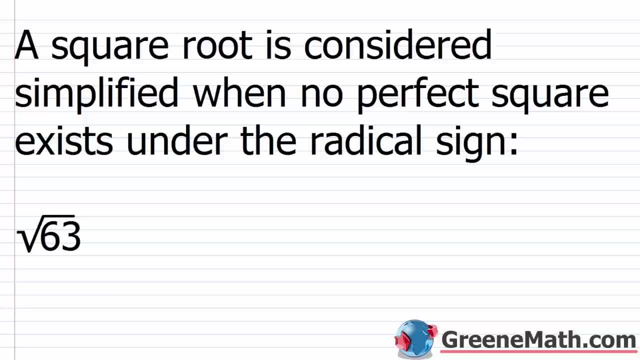 Remember all to use the product rule for radicals. That's kind of the first type of problem you're going to encounter in this section. Then you're going to kind of move on and talk about simplifying radicals. So this is where you've got to take this rule that you just learned and kind of apply it. So a square root is considered simplified. 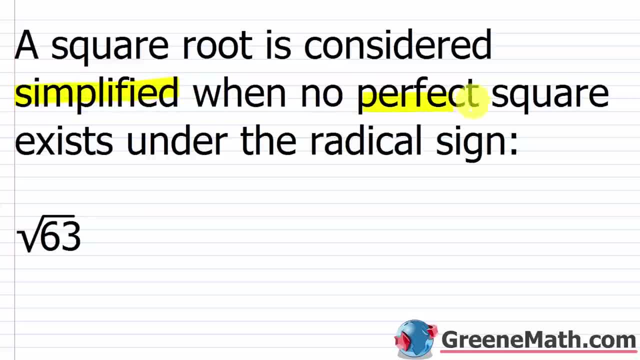 Okay. Simplified when no perfect square exists under the radical sign. Okay. So what do we mean when we say a perfect square? Remember a number, a number has to be a perfect square if its square root is a rational number. So four is a perfect square because its square root two is a rational number. One fourth is a perfect square because its square root one half is a rational number. So what I'm going to do here in each case is I'm going to break down the number under the square root symbol and I'm going to be looking for perfect squares. 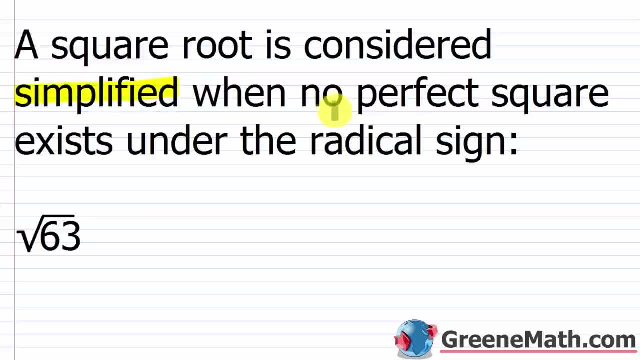 learned and kind of apply it. So this is where you've got to take this rule that you just learned. So what do we mean when we say a perfect square? Remember, a number is a perfect square if it's square root is a rational number. A number is square root if it's square root is a. 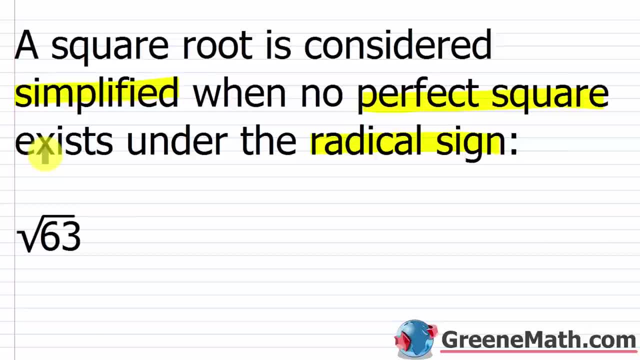 rational number. Therefore, it's a perfect square. So what you're going to do is you're going to get the seeing this parallel sequence plot and you're going to get the story line that you want to get to wrap it around. So 4 is a perfect square because it's square root. 2 is a rational number. 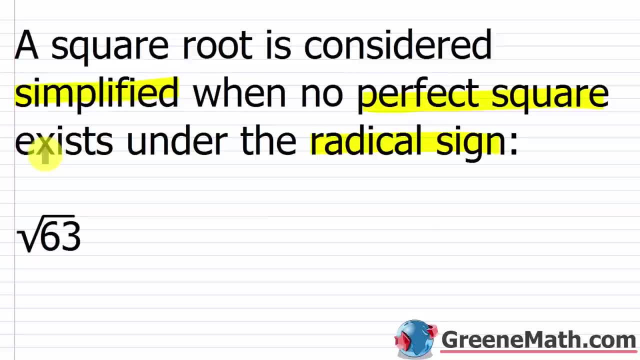 One fourth is a perfect square because it's square root one half, which means that two times that is what's going to make change. if I can make side is a rational number. So what I'm gonna do here in each case is I'm going to 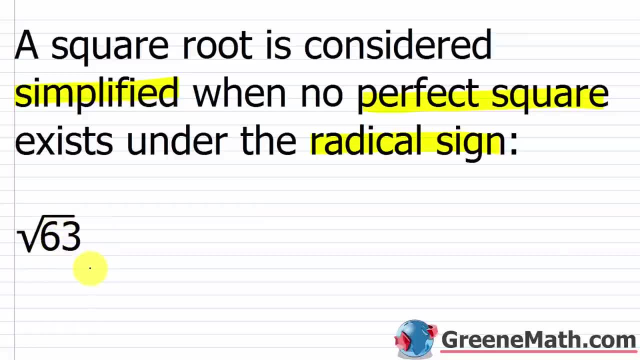 break down the number under the square root symbol and I'm gonna be looking for perfect squares in its factorization. So let's take a look at this kind of first one where we have the square root of 63.. So you can go off to the side and make a 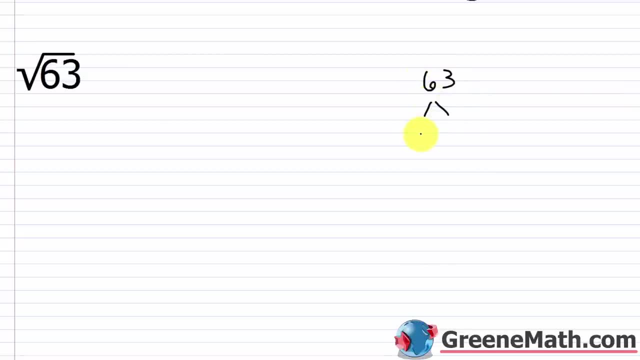 factor tree if you want and say: okay, well, 63 is what it's 9 times 7.. I know 7 is prime and 9 is 3 times 3.. So 9 is a perfect square. so, using my product rule for radicals, I could break this down into the square root of 9 times 7 and 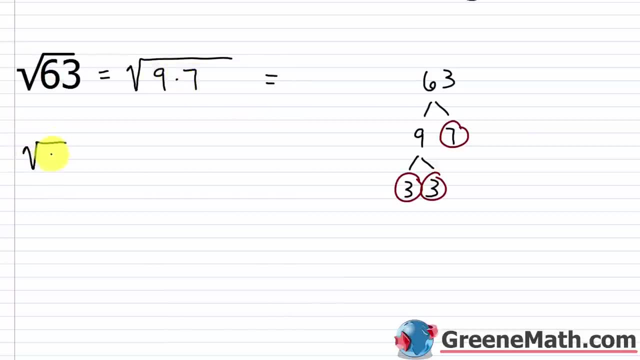 then I could further break it down into the square root of 9 times the square root of 7.. Now we just showed that 9 is a perfect square, right, We know it's 3 times 3, so the square root of 9 is 3, so I could put this as equal to. 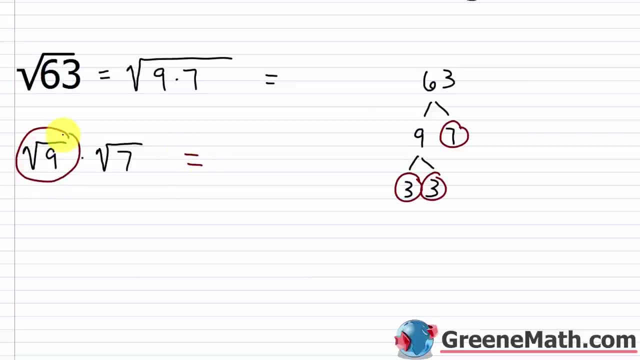 this guy right here is just going to simplify to three. So I'm just going to write a three instead of the square root of nine, And then it's multiplied by the square root of seven. So then times the square root of seven. So this three times the square root of seven is considered. 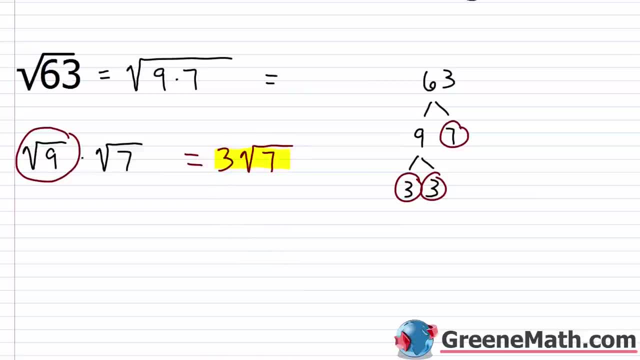 simplified. If we look at what's underneath our square root symbol. now seven. you can't factor seven any further. It's a prime number, right? So seven is not a perfect square. So no perfect square exists under that radical sign, unless you were to consider something like one which 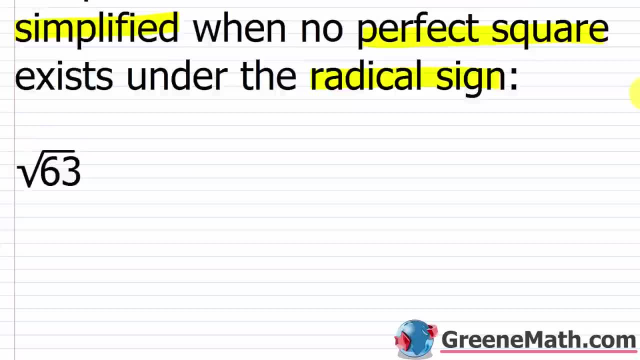 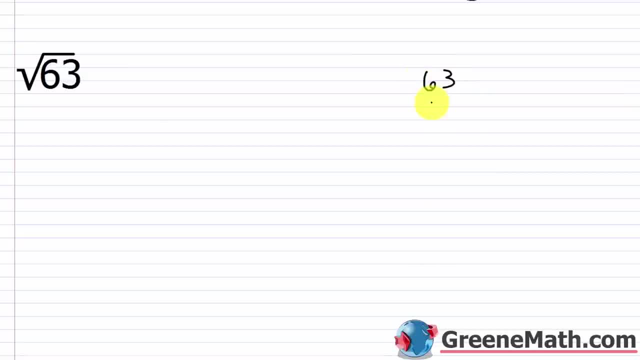 factorization. So let's take a look at this kind of first one where we have the square root of 63. So you can go off to the side and make a factor tree if you want and say okay well 63 is what? It's 9 times 7. I know 7 is prime and 9 is 3 times 3. So 9 is a perfect square. So using my product rule for radicals I could break this down into the square root of 9 times 7 and then I could further break it down into the square root of 9 times the square root of 7. Now we just showed that 9 is a perfect square. We know it's 3 times 3 so the square root of 9 is 3. So I could put this as equal to this guy right here is just going to simplify to 3. So I'm just going to write a 3 instead of the square root of 9 and then it's multiplied by the square root of 7. 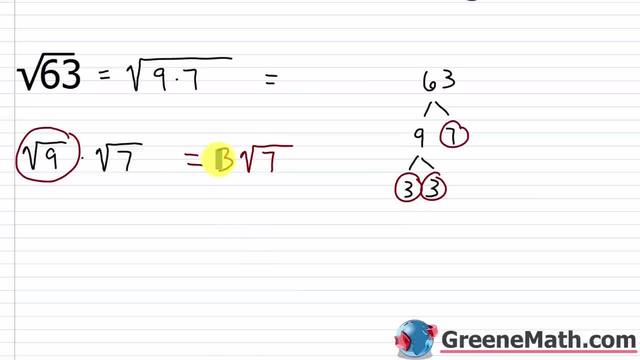 So then times the square root of 7. So this 3 times the square root of 7 is considered simplified. If we look at what's underneath our square root symbol now 7 you can't factor 7 any further. It's a prime number right. So 7 is not a perfect square. So no perfect square exists under that radical sign unless you were to consider something like 1 which we really can't do anything with that right. So we would say 3 times the square root of 7 is the simplified version of the square root of 7. So we can't do anything with that. So we can't do anything with that. 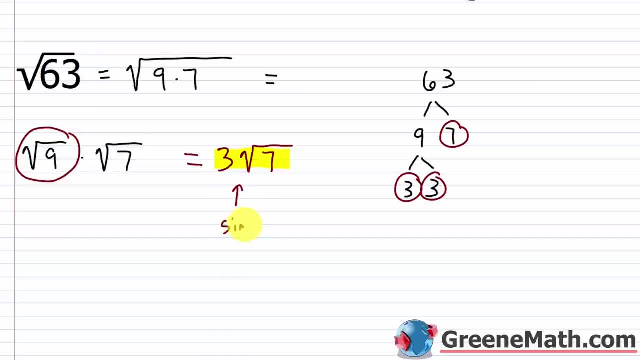 of the square root of 63, so this is simplified. 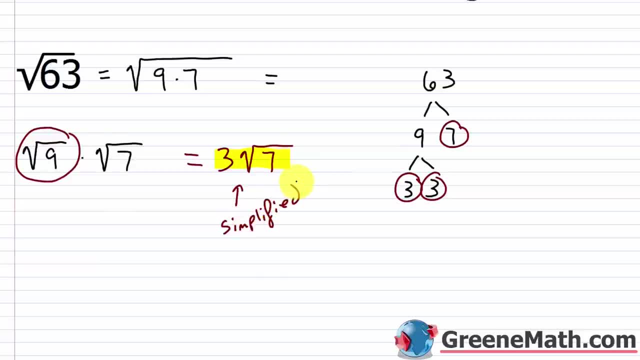 Now to prove that to yourself, you could punch up square root of 63 in a calculator, and then also punch up three times the square root of seven on a calculator, and you're gonna see that you're gonna get the exact same value. 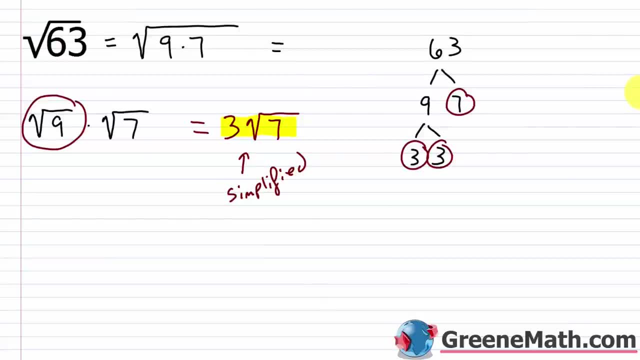 Now before I move forward, I wanna show you kind of an alternative way to do this. 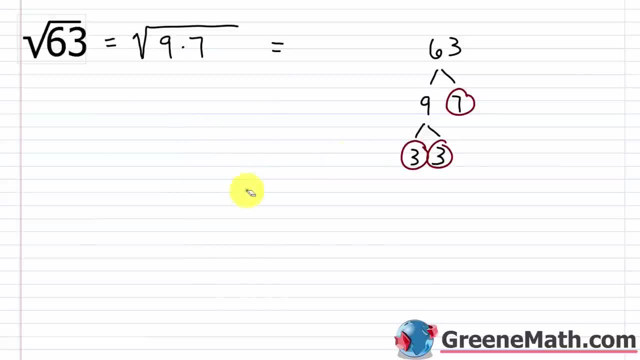 So we've seen this method, let me kind of erase this, and I wanna show you something else you can do. 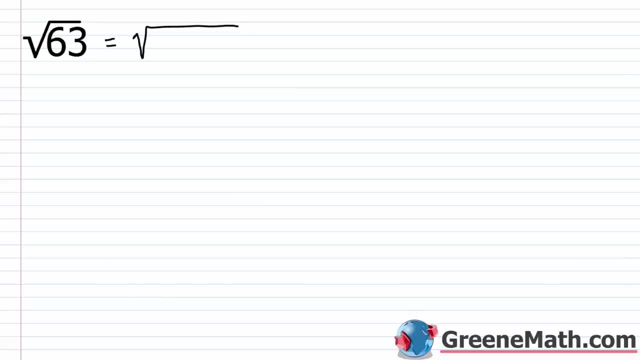 This is very, very common. So if I have the square root of 63, I can kind of factor it under my square root symbol that I created. So I could say, okay, well, I know it's nine times seven. 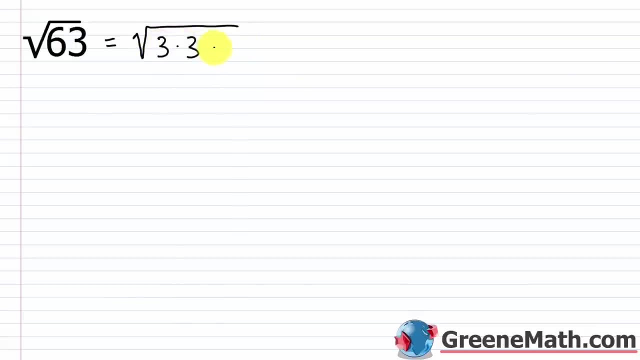 Nine is three times three, so I would put three times three times seven. 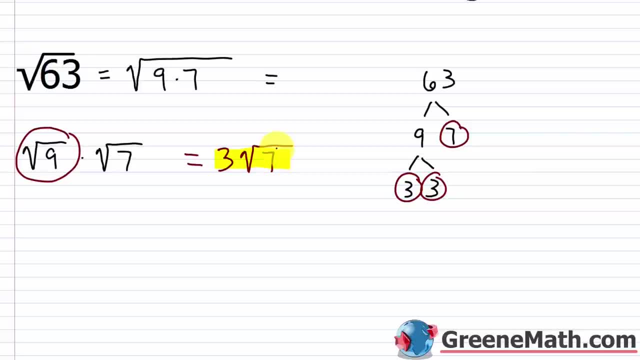 we really can't do anything with that, right? So we would say three times: the square root of seven is the simplified version of the square root of 63. So this is simplified. Now, to prove that to yourself, you could punch up square root of 63 in a calculator. 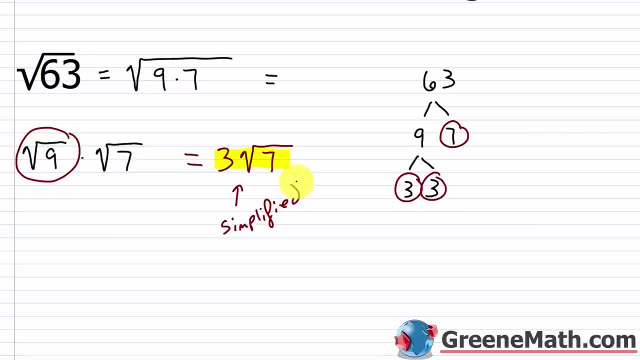 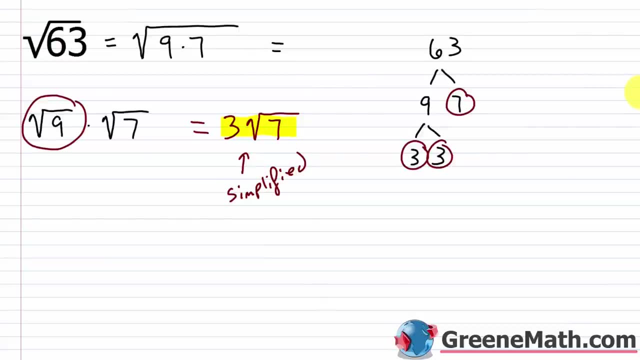 and then also punch up three times the square root of seven on a calculator And you're going to see that you're going to get the exact same value. Now, before I move forward, I want to show you kind of an alternative way to do this. 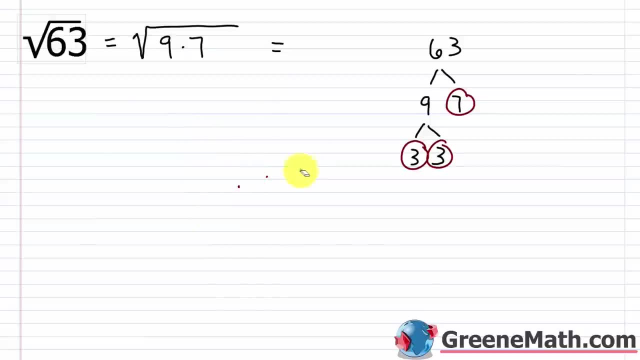 So we've seen this method. let me kind of erase this And I want to show you something else you can do. This is very, very common. So if I have the square root of 63, I can kind of factor it under my square root symbol that I create. So I could say: okay, well, I know it's nine times. 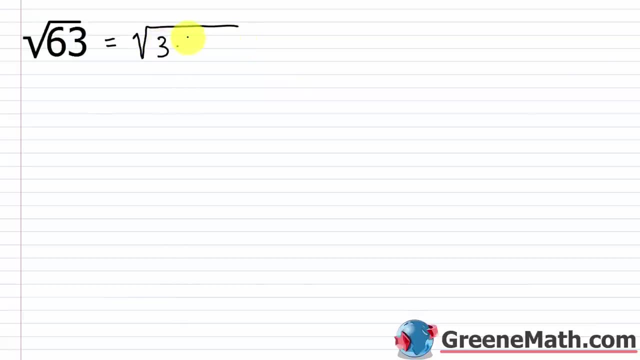 seven nine is three times three. So I would put three times three times seven. So, without making a factor tree, I just kind of factor it underneath the symbol. And then what I do is I look for pairs of numbers. In this case I have a pair, I have one pair of threes. 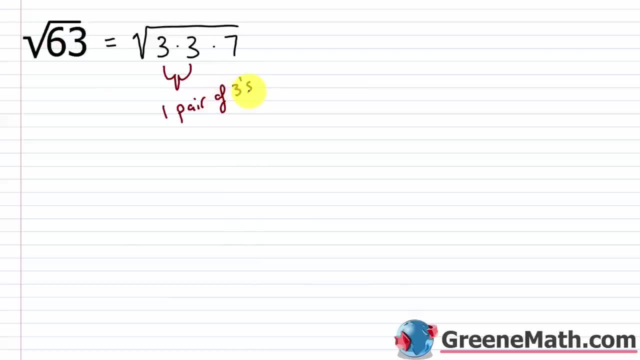 So for each pair that I have, I can pull that outside of my square root symbol, right? Because the square root of three times three would obviously be three. So if I have a pair of numbers I can pull one of those out. So for each pair I pull one out. So, in other words, 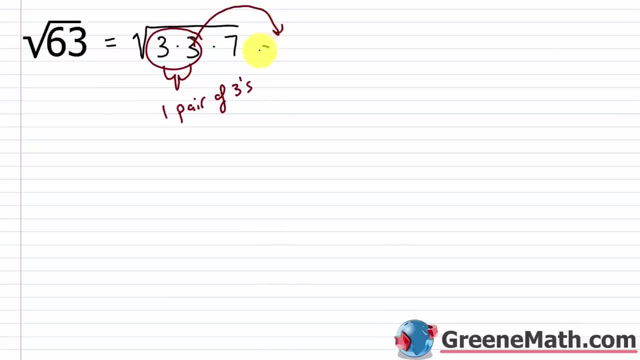 I would just circle this and say I can pull one of those out and say I have three times the square root of seven. So it's kind of an alternative way to look at that. I know that you'll probably see that in some of your textbooks and it's a common strategy that a lot of teachers will show you when. 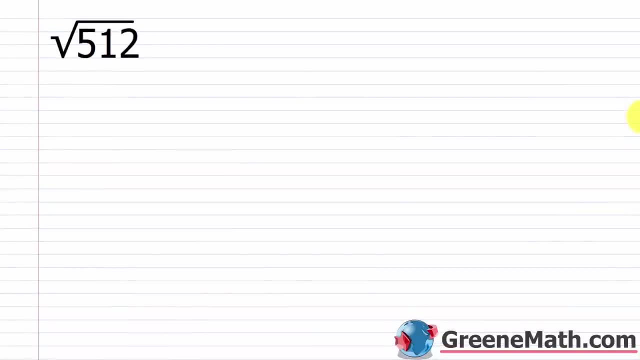 they're covering this in class. All right, let's take a look at another one. So let's say that you ran across something like the square root of 512.. So if you're like myself, you know two up to like the 20th power because you use it all the time. But in an algebra one course, you probably 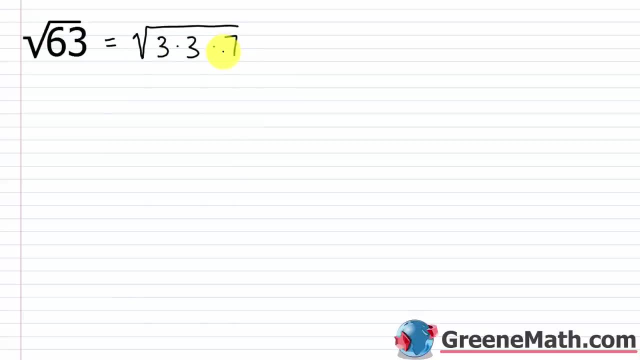 So without making a factor tree, I just kind of factor it underneath the symbol, and then what I do is I look for pairs of numbers. In this case, I have a pair, I have one pair, I have a pair of threes. So for each pair that I have, I can pull that outside of my square root symbol, right? Because the square root of three times three would obviously be three. 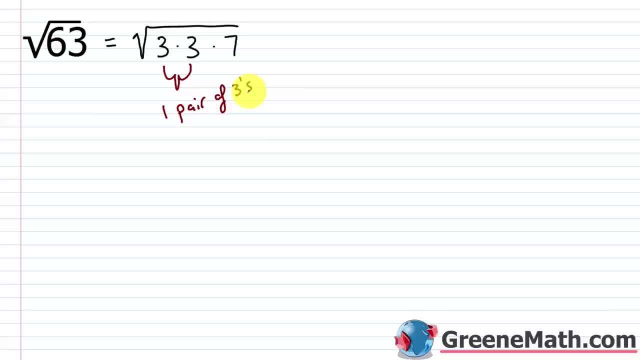 So if I have a pair of numbers, I can pull one of those out. So for each pair, I pull one out. So in other words, I would just circle this and say, I can pull one of those out, 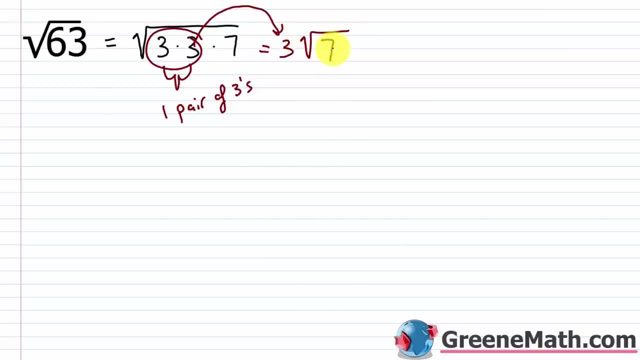 and say I have three times the square root of seven. So it's kind of an alternative way to look at that. I know that you'll probably see that in some of your textbooks, and it's a common strategy that a lot of teachers will show you when they're covering this in class. 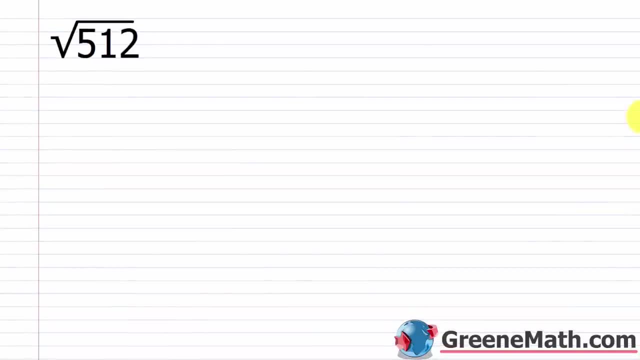 All right, let's take a look at another one. So let's say that you ran across something 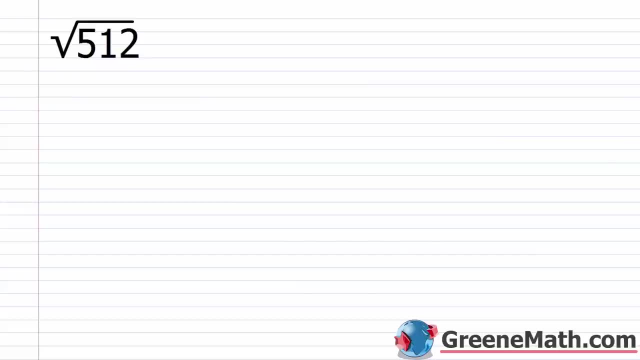 like the square root of 512. So if you're like myself, you know two up to like the 20th power, because you use it all the time. But in an Algebra I course, you probably only know stuff like two up to the sixth or seventh power. 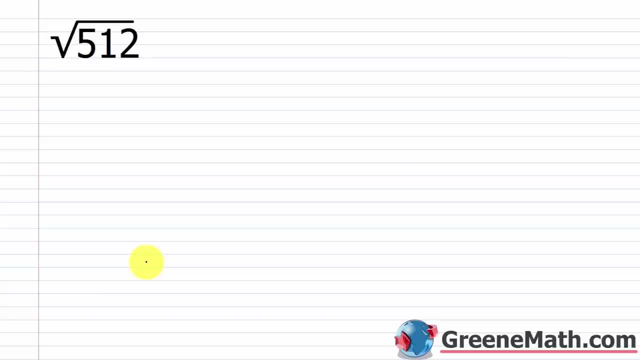 512 happens to be two to the ninth power, but you might not know that. 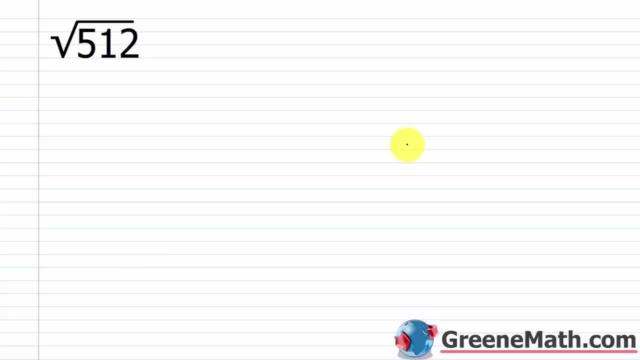 So if you didn't know it, again, you've got to have some method, like a factor tree to kind of break the number down. 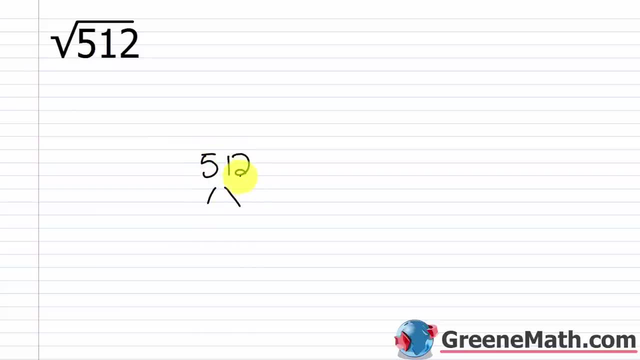 So let's say I said 512 is divisible by two. It's also divisible by four, right? Because it ends in 12. So I can say this is 128 times four. Then four is what? It's two times two. 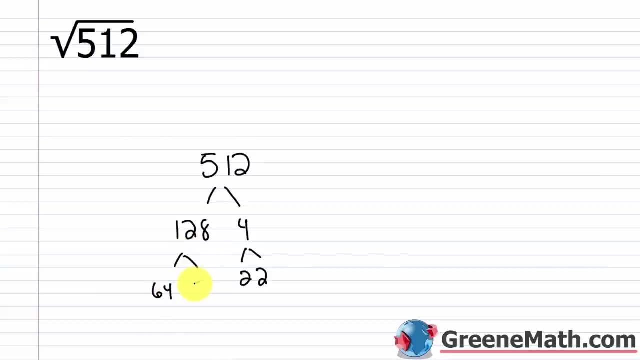 And 128 is 64 times two. Now, once you start getting into some numbers where you can recognize that it's two to a certain power, 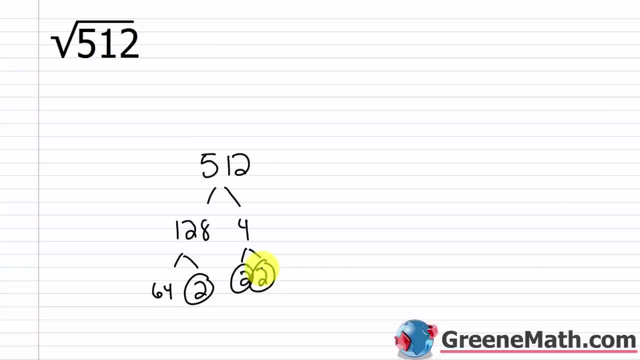 like we know 64 is two to the sixth power. Even if you didn't know that, once you break down 64 into what, 32 times two, you should know that this is two to the fifth power. 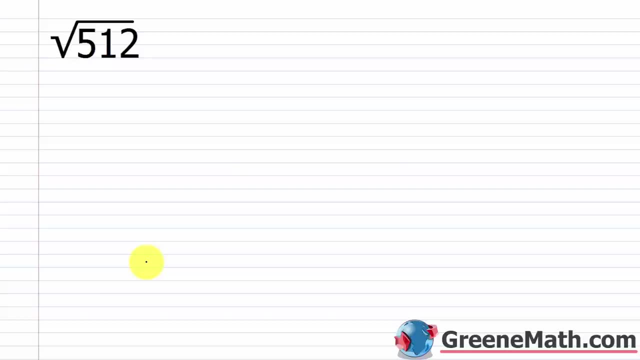 only know stuff like two up to the sixth or seventh power. 512 happens to be two to the ninth power, but you might not know that. So if you didn't know it again, you've got to have some method like a factor tree to kind of break the number down. So let's say I said 512. 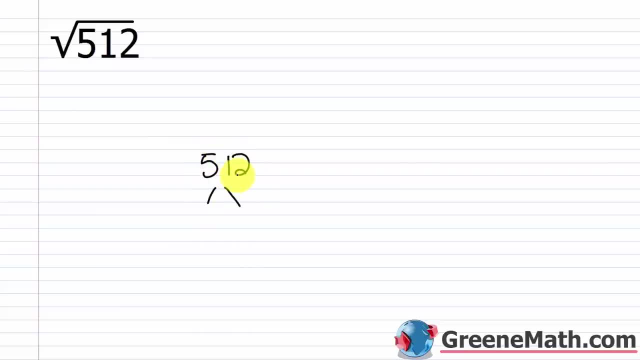 512.. is divisible by 2.. It's also divisible by 4, right, because it ends in 12.. So I can say: this is 128 times 4.. Then 4 is what It's 2 times 2. And 128 is 64 times 2.. Now, once you start getting, 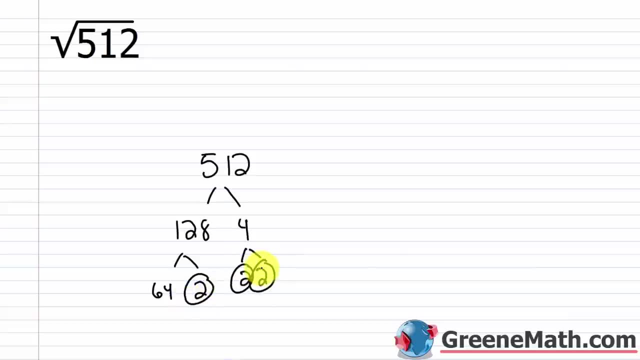 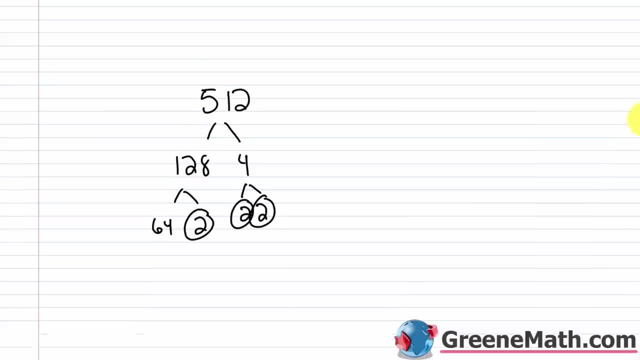 into some numbers where you can recognize that it's 2 to a certain power. like we know, 64 is 2 to the 6th power. Even if you didn't know that, once you break down 64 into what? 32 times 2,. 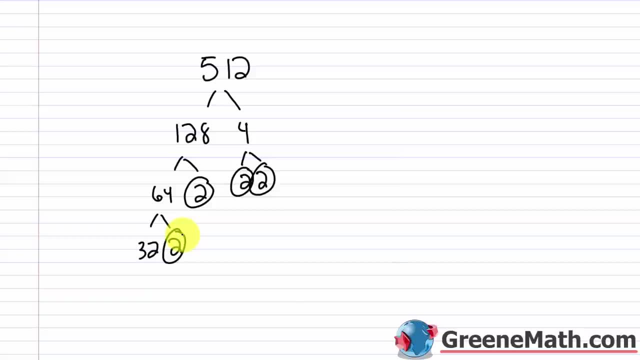 you should know that this is 2 to the 5th power, So you should be able to stop and say, okay, well, if this is 2 to the 5th power and I have 1,, 2,, 3,, 4 more, well then really the whole thing would. 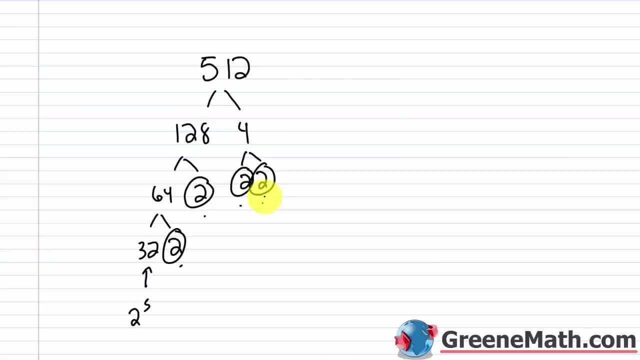 be 2 to the power of 5 plus 4, or 2 to the 9th power. So let me erase this And once you realize that there's a few different ways, you can kind of take that. So let's take a look at this. 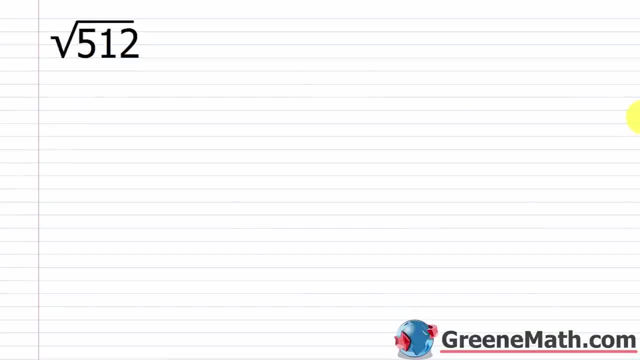 Let's tackle something like this So kind of the traditional way or the way you just saw a minute ago. you can, under the square root symbol, write out 9 factors of 2.. So 2 times 2, times 2. 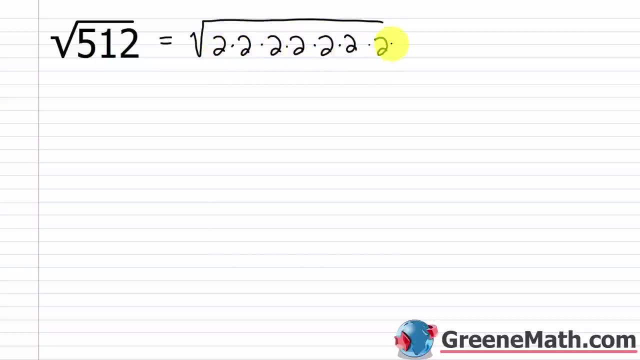 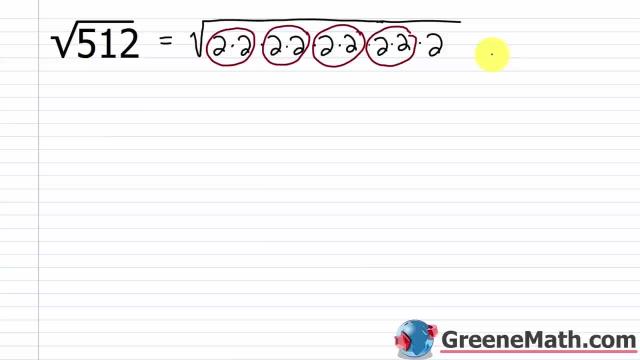 here's a 4th. For each pair you're going to pull out 1,, 2, right, Because the square root of 2 times 2 would be 2, right Square root of 4 is 2.. So this is equal to, again, for each 1, you're pulling. 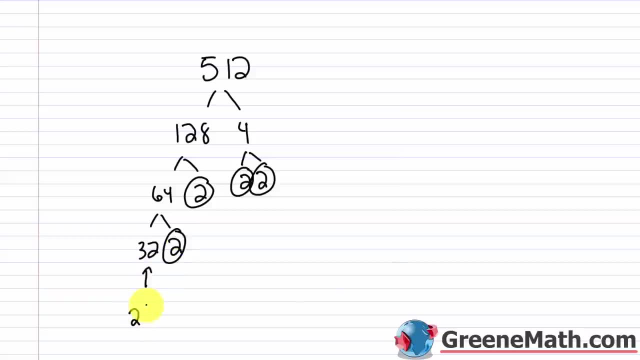 So you should be able to stop and say, okay, well, if this is two to the fifth power and I have one, two, three, four more, well then really the whole thing would be two to the power of five plus four or two to the ninth power. 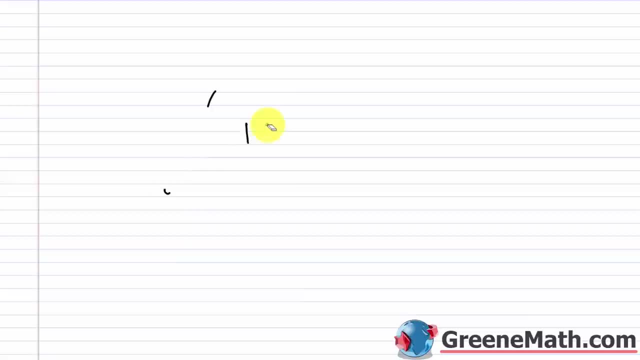 So let me erase this. And once you realize that, there's a few different ways you can kind of tackle something like this. 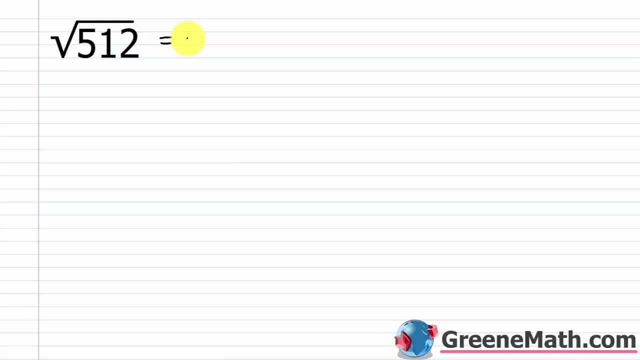 So kind of the traditional way or the way you just saw a minute ago, you can under the square root symbol, write out nine factors of two. 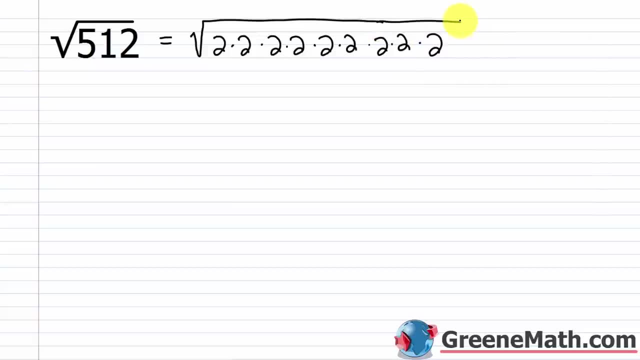 times two times two and then times two. So nine factors of two. 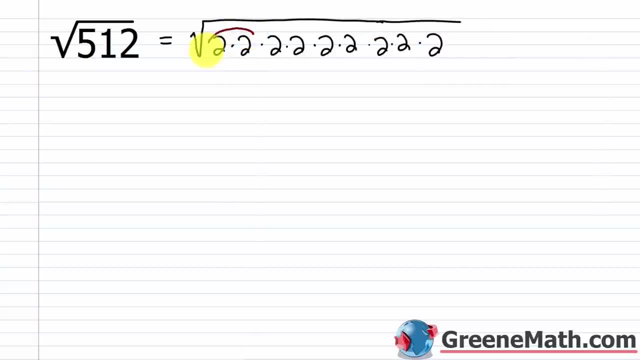 Then for each pair of twos, so here's one, here's a second, here's a third, here's a fourth. 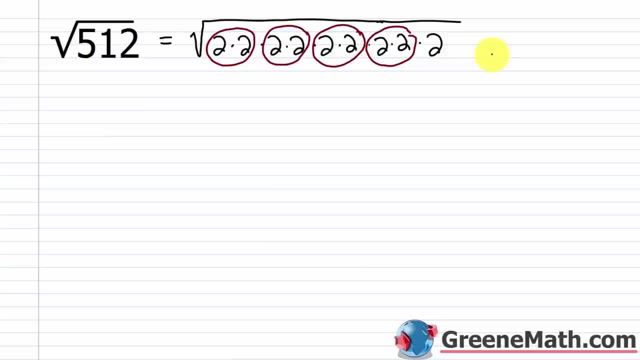 For each pair, you're gonna pull out one, two, right? Cause the square root of two times two would be two, right? Square root of four is two. So this is equal to, again, for each one, you're pulling out one. 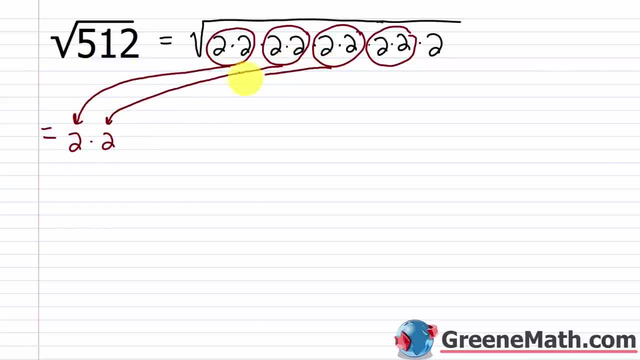 So this is two times two times two times two. 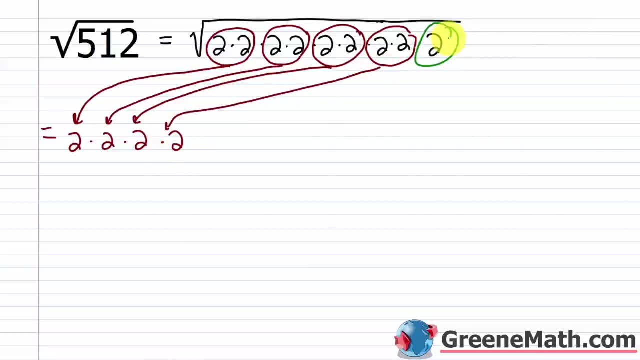 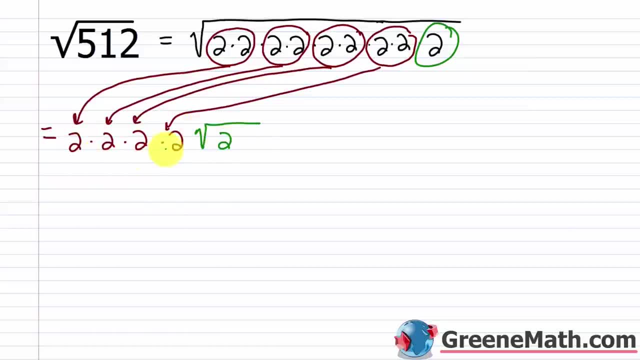 we know that two to the fourth power or two times two times two times two is 16. 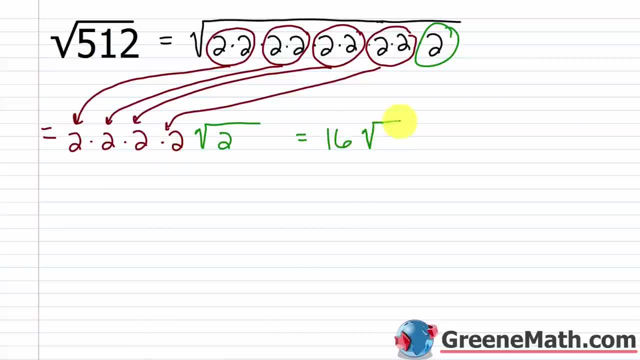 So this would simplify to 16 times the square root of two. 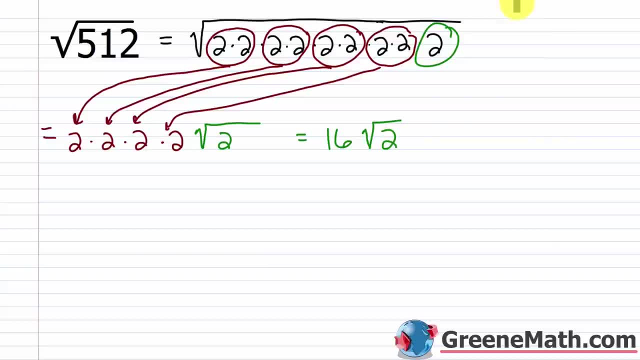 Is there anything else I can do to simplify this? No, there's not. The square root of two is not gonna be able to be simplified any further because under that square root symbol, there's no more perfect squares, right? Two is a prime number. It's not gonna factor any further. 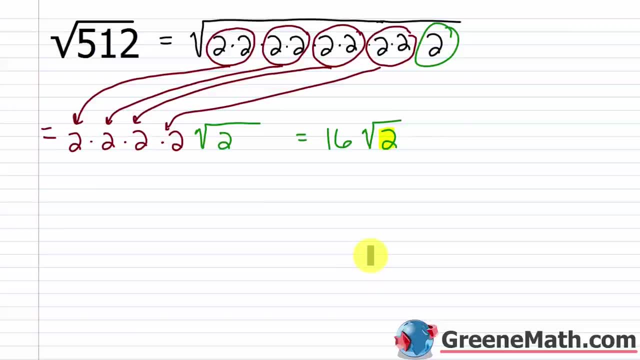 And two is just simply not a perfect square. So there's nothing else we can do. 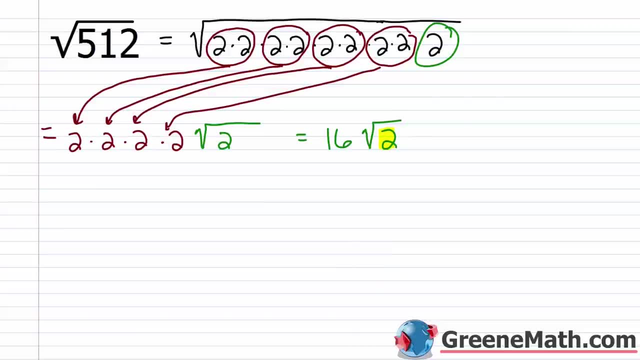 Now, another way to kind of tackle this problem, you're gonna get the same result either way, but it's just kind of a quicker way to do it. If I saw something like the square root of 512, 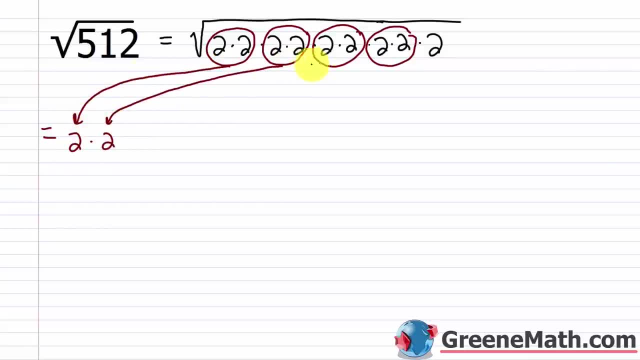 out 1.. So this is 2 times 2, times 2, times 2.. Then what's left inside is a lonely 2.. So then, all this times, the square root of 2.. We know that 2 to the 4th power, or 2 times 2,. 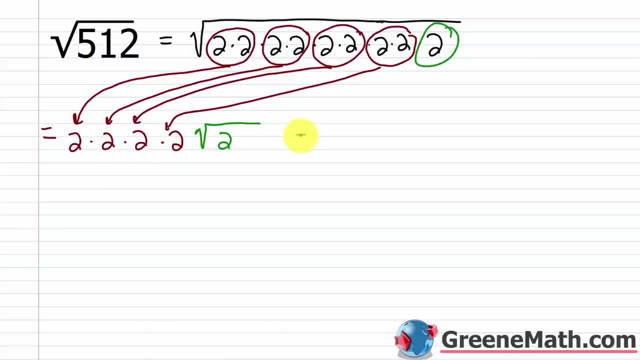 times 2, times 2, is 16.. So this would simplify to 16 times the square root of 2.. Is there anything else I can do to simplify this? No, there's not. The square root of 2 is not going to be able to. 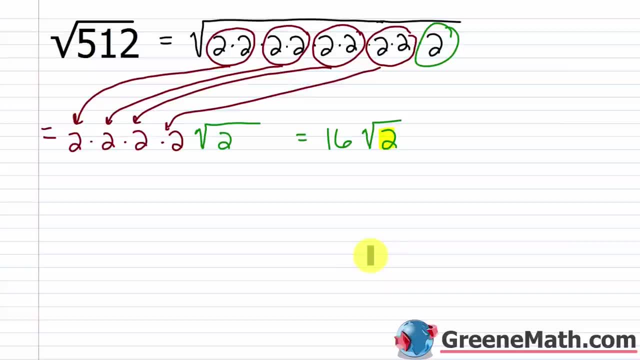 be simplified any further, because under that square root symbol there's no more perfect squares right. 2 is a prime number, it's not going to factor any further, and 2 is just simply not a perfect square. So there's nothing else we can do Now. another way to kind of tackle this. 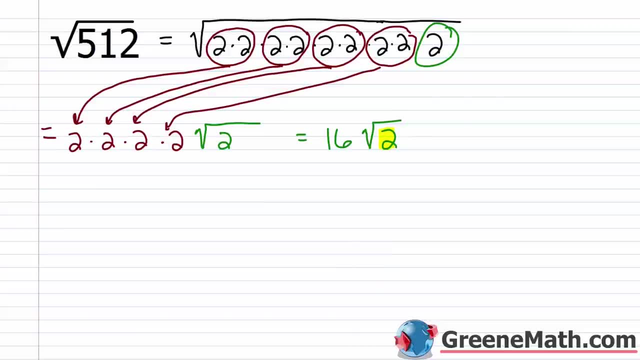 problem you're going to have to do, is you're going to have to do, is you're going to have to get the same result either way, but it's just kind of a quicker way to do it If I saw something like the square root of 512, and I recognize very quickly that this is 2 to the 9th power. 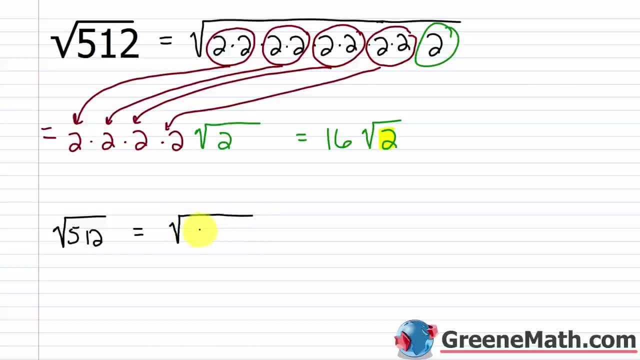 you could write this as the square root of 2 to the 9th power. Now, later on, when we get to fractional exponents, you're going to really be able to simplify this quickly, because I'm going to teach you that the square root symbol is like raising something to the one-half. 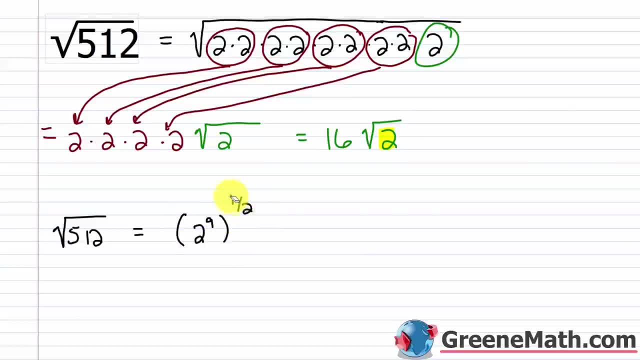 power. okay, And we'll get to this later, but I'm not trying to go too far ahead, But for right now we're stuck with kind of this symbol. So we have the square root of 2 to the 9th power. 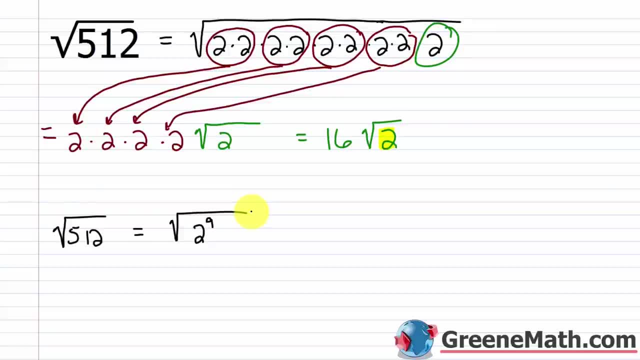 Now, if I had an even exponent on that 2, something like 2 to the 8th power, so let's rewrite this as square root of 2 to the 8th power times square root of 2 to the first power, or just 2,. 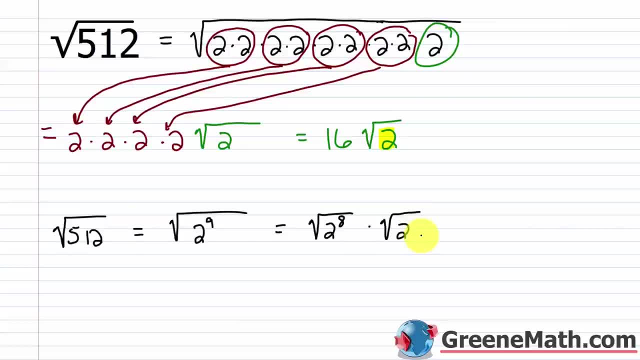 right. Everything is equal here. I haven't changed the value of anything. Square root of 2 to the 8th power would be what. Well, think about what I just taught you a minute ago. If I had 2 to the 8th power and this was raised to the power of one-half, well, I would. 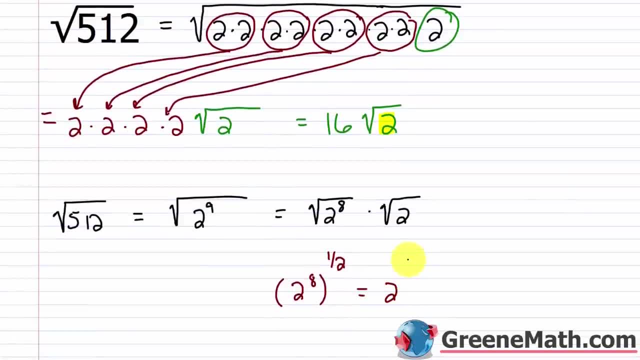 multiply exponents. keep the base the same. This is 2 raised to the power of 8 divided by 2, or 2 to the 4th power. 2 to the 4th power we already know is 16.. And again it's getting a little far. 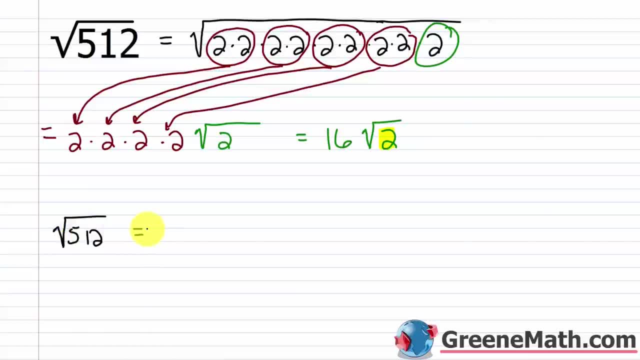 and I recognize very quickly that this is two to the ninth power, you could write this as the square root of two to the ninth power. 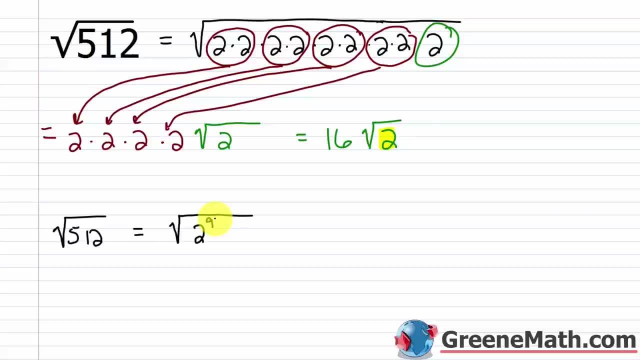 Now, later on, when we get to fractional exponents, you're gonna really be able to simplify this quickly, because I'm gonna teach you that the square root symbol is like raising something to the one half power, okay? And we'll get to this later, 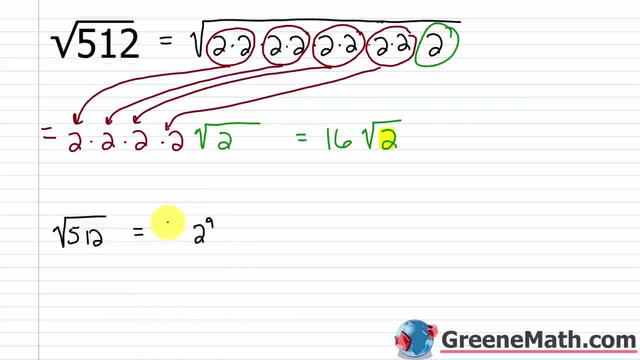 but I'm not trying to go too far ahead. But for right now, we're stuck with kind of this symbol. 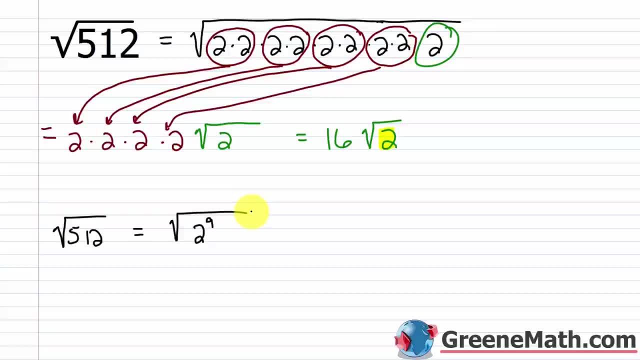 So we have the square root of two to the ninth power. Now, if I had an even exponent on that two, something like two to the eighth power, so let's rewrite this as square root of two to the eighth power times square root of two, to the first power or just two, right? Everything is equal here. I haven't changed the value of anything. 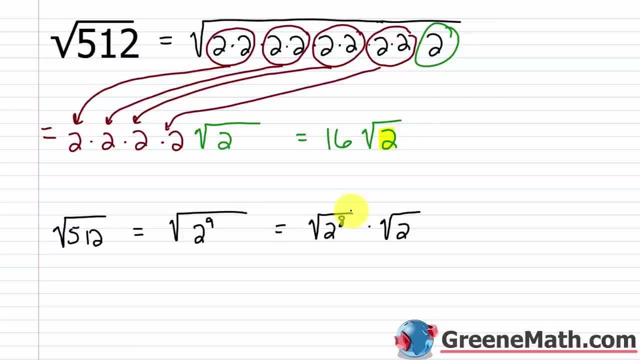 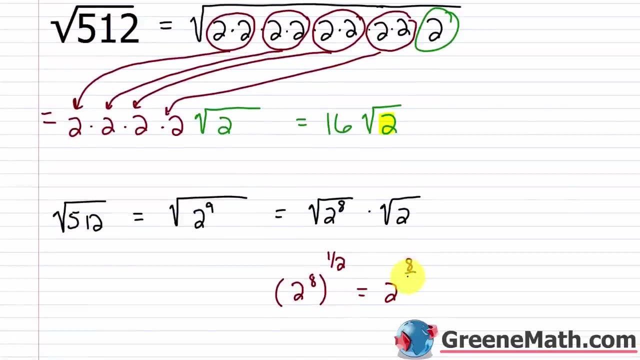 So the square root of two to the eighth power would be what? Well, think about what I just taught you a minute ago. If I had two to the eighth power, and this was raised to the power of one half, well, I would multiply exponents, keep the base the same. This is two raised to the power of eight divided by two, or two to the fourth power. Two to the fourth power we already know is 16. 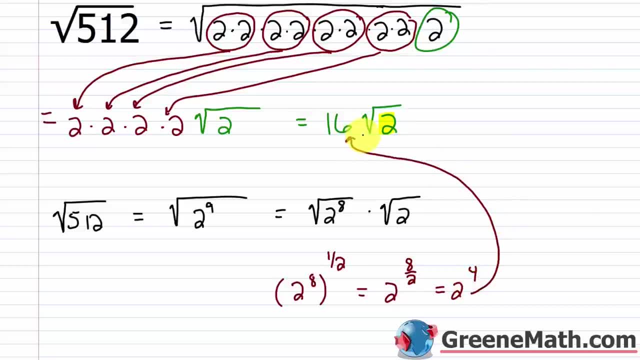 And again, it's getting a little far ahead of where we are at this point, but I just want you to realize that there's gonna be some strategies coming up that are going to really reduce the amount of work 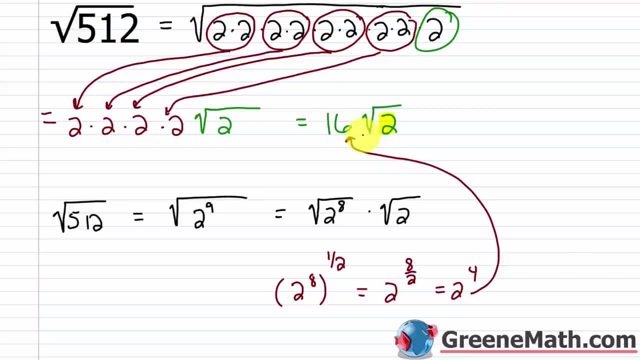 you have to do with these problems. You know, another thing you can do 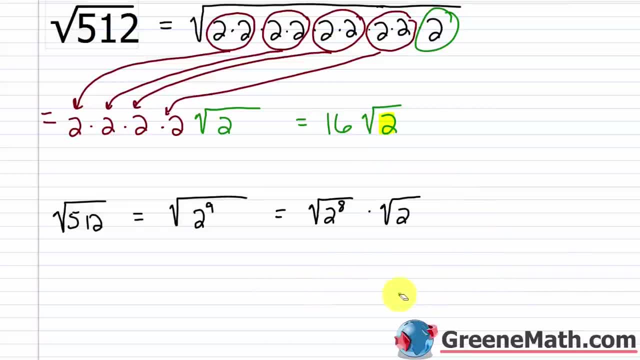 if you didn't have kind of the exponent trick under your belt yet, you could just really think about, okay, well, how could I break two to the eighth power down 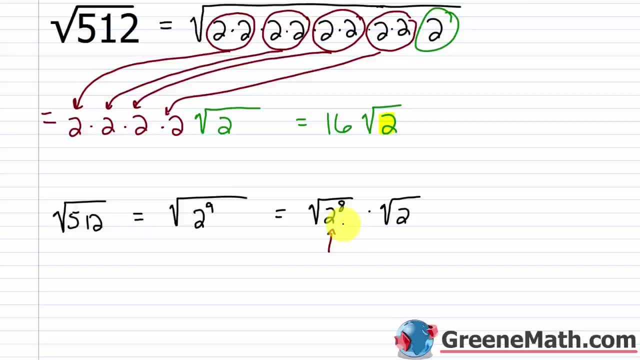 into two to some power squared that would get me to two to the eighth power, right? You could realize that this is two to the fourth power, that amount squared, and then we take the square root of that. 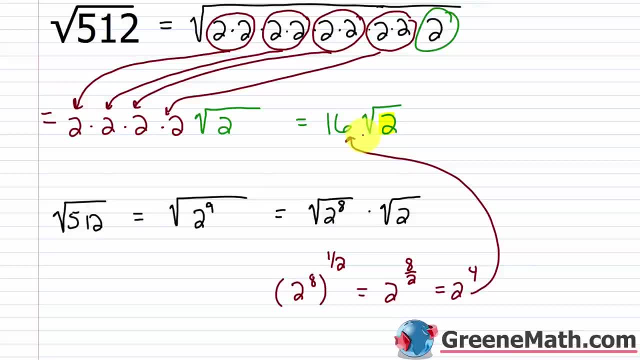 ahead of where we are at this point, but I just want you to realize that there's going to be some strategies coming up that are going to help you get to the point where you're going to be able to get to the point where you're going to be able to get to the point where you're going to be able to. 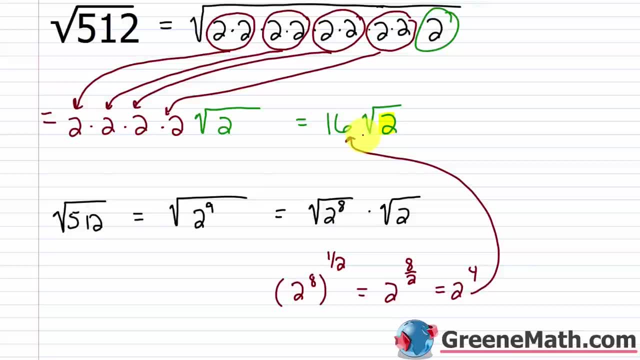 sum things up that are going to really reduce the amount of work you have to do with these problems. You know another thing you can do. if you didn't have kind of the exponent trick under your belt yet, you could just really think about: okay, well, how could I break 2 to the 8th power? 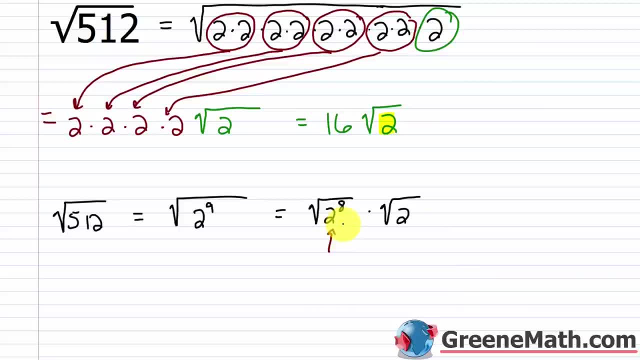 down into 2 to some power squared, that would get me to 2 to the 8th power. right, You could realize that this is 2 to the 4th power, that amount squared, and then we take the square root of that. 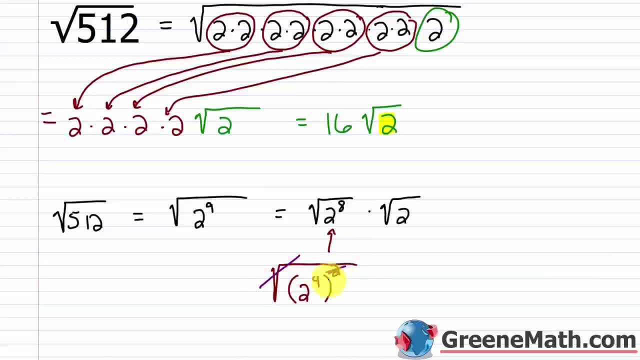 Well then, we learned in the last video that what we're going to do is we're going to get to the in the last lesson, that this cancels with this and I'm left with 2 to the 4th power, So kind of. 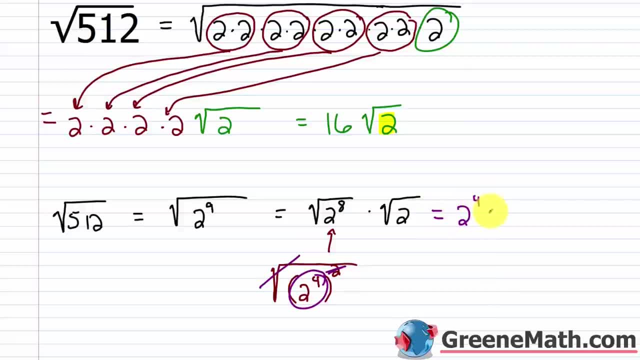 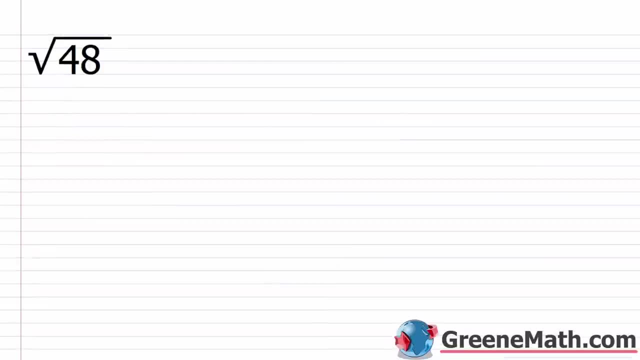 any way you think about this, this would be 2 to the 4th power times the square root of 2, or again 16 times the square root of 2 as your simplified answer. All right, what about something like the: 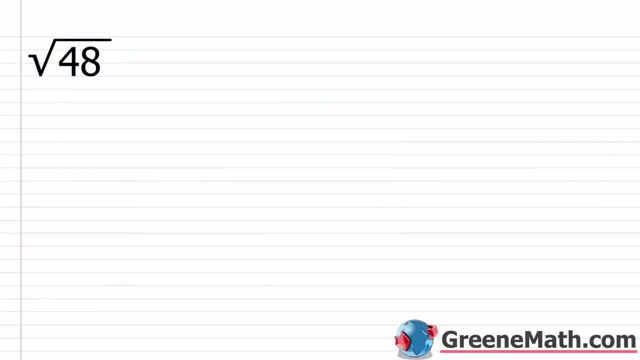 square root of 48?? Well, 48,. I can kind of do that in my head, So let me kind of just write this as the square root of. I know I could do 4 times 12, but one of the things about 12 is it's also got a. 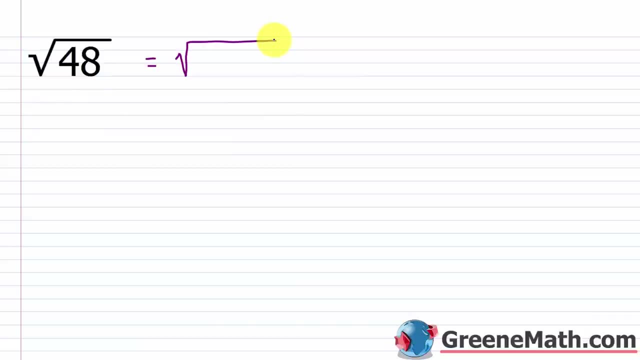 4.. So I've already got a 4 times a 4 there, So I could do what I could do 16 times 3.. So I could do square root of 16 times 3.. I know, 16 is a perfect square. This is a perfect square Square. 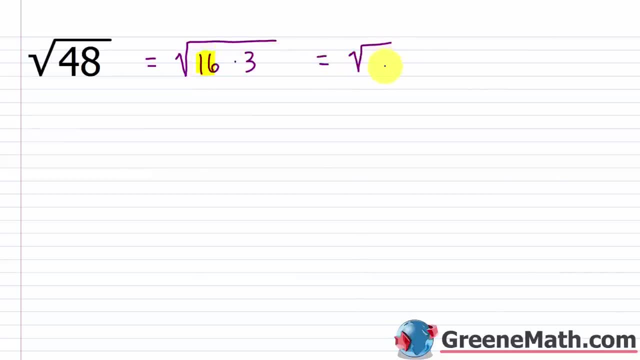 root of 16 is 4.. So I could write this as the square root of 16 times the square root of 3, and then, bam, I've got my answer. I know, square root of 16 is 4 times the square root of 3.. Now 3 is a prime number. It can't be. 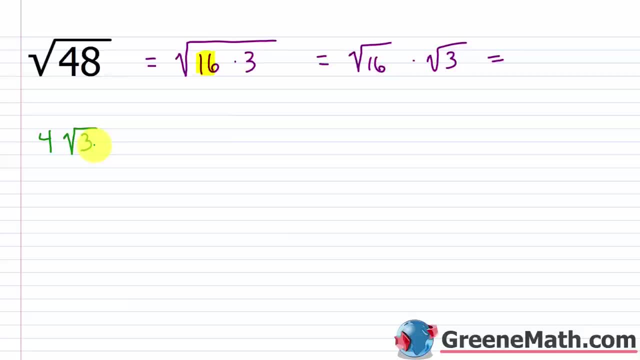 factored any further and it's not a perfect square. So this is as simple as we can make this And again, if you wanted to do this the other way, you could say: okay, well, the square root of 48. 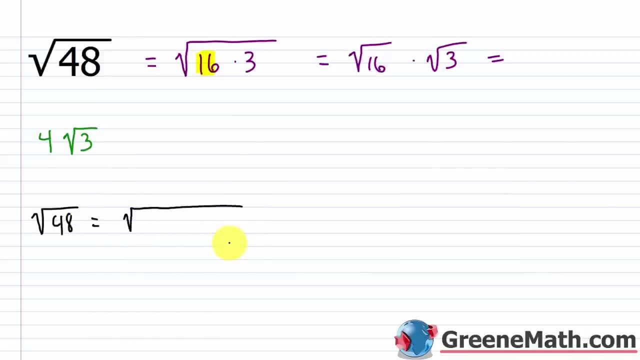 is equal to what The square root of you could do 4 times 4 times 3.. And then again, if you have a pair of 4s, one of those is going to go outside of the square root symbol, And then you'll just have the square root of 3. that's left. 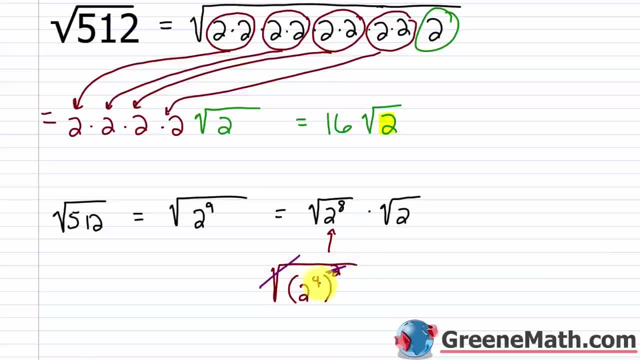 Well, then we learned in the last lesson that this cancels with this, and I'm left with two to the fourth power. So kind of any way you think about this, this would be two to the fourth power times the square root of two, or again, 16 times the square root of two as your simplified answer. 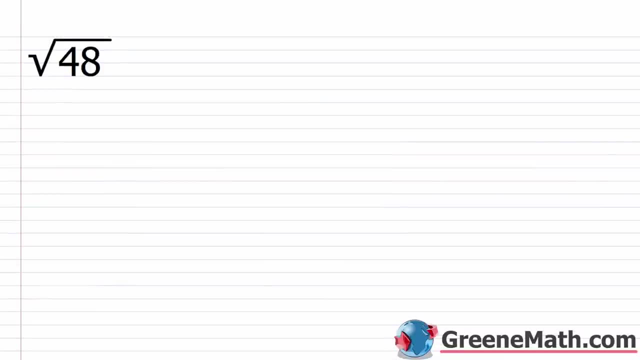 All right, what about something like the square root of 48? Well, 48, I can kind of do that in my head. So let me kind of just write this as the square root of, I know I could do four times 12, but one of the things about 12 is it's also got a four. So I've already got a four times a four there. So I could do what? I could do 16 times three. 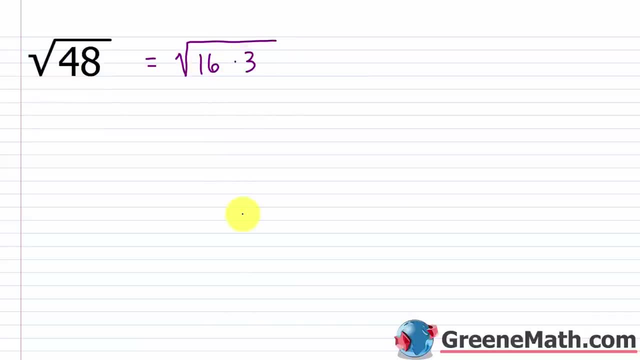 So I could do square root of 16 times three. I know 16 is a perfect square. This is a perfect square. Square root of 16 is four. So I could write this as the square root of 16 times the square root of three, and then bam, I've got my answer. 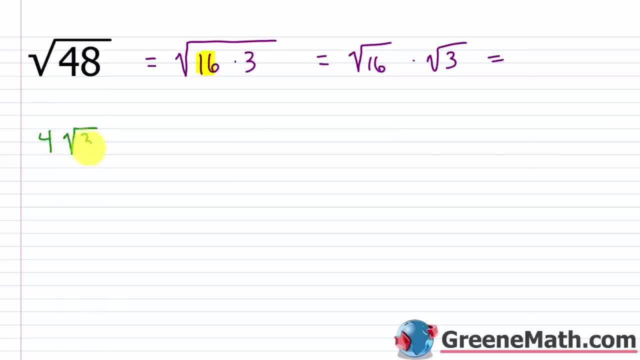 I know square root of 16 is four times the square root of three. 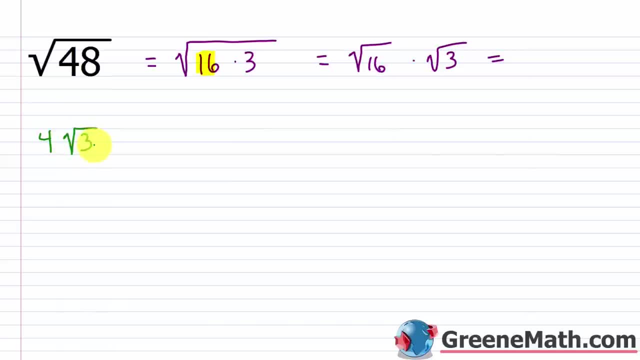 Now, three is a prime number. It can't be factored any further, and it's not a perfect square. 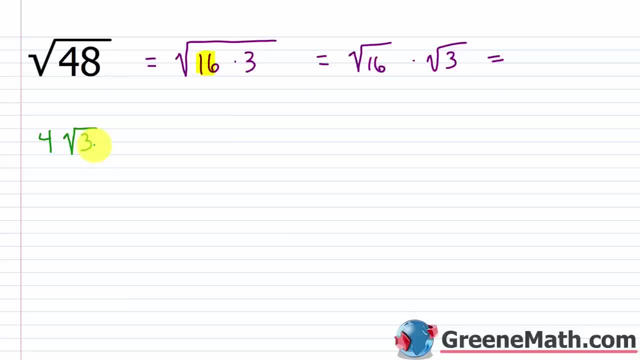 So this is as simple as we can make this. And again, if you wanted to do this the other way, you could say, okay, well, 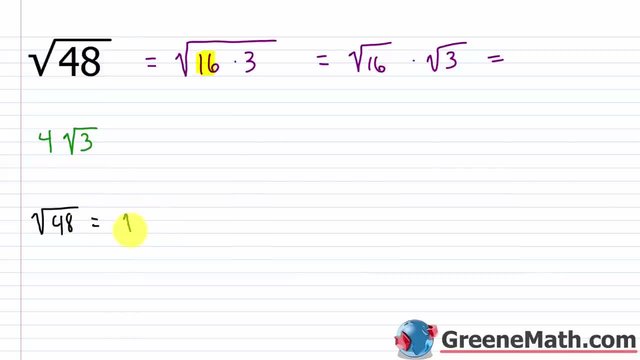 the square root of 48 is equal to what? The square root of, you could do four times four times three. 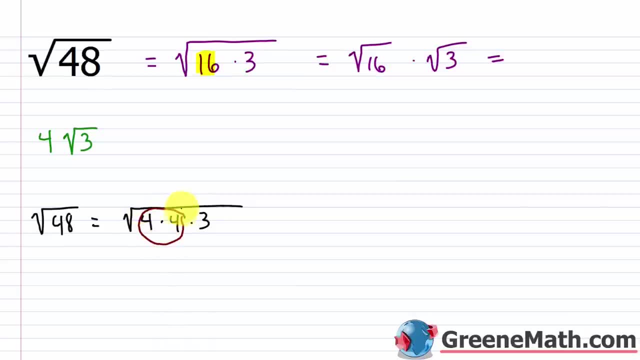 And then again, if you have a pair of fours, one of those is gonna go out. It's gonna go outside of the square root symbol. And then you'll just have the square root of three that's left. 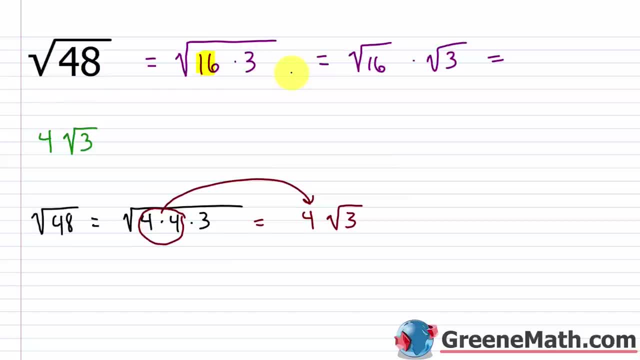 So kind of either way you wanna look at this, you're gonna get the same answer. 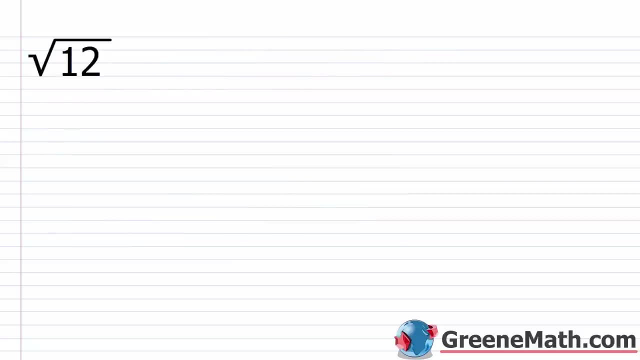 What about the square root of 12? Well, 12, again, I can break that down into the square root of four times three. 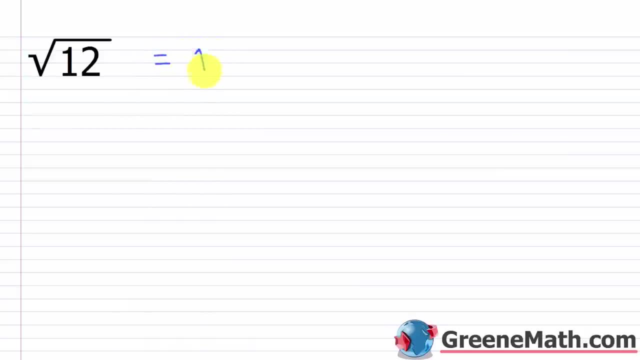 The square root of four is two. So this would be equal to the square root, I'm gonna do, of four times three. 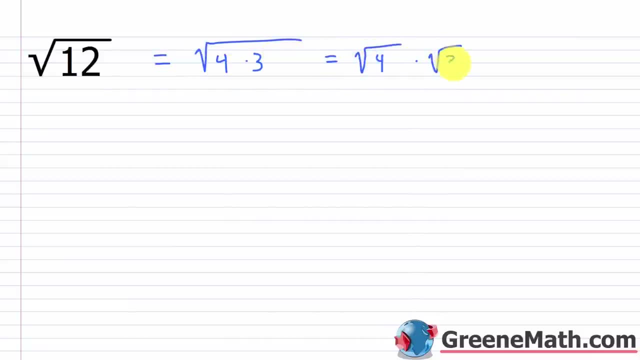 And then I'll write the square root of four times the square root of three. 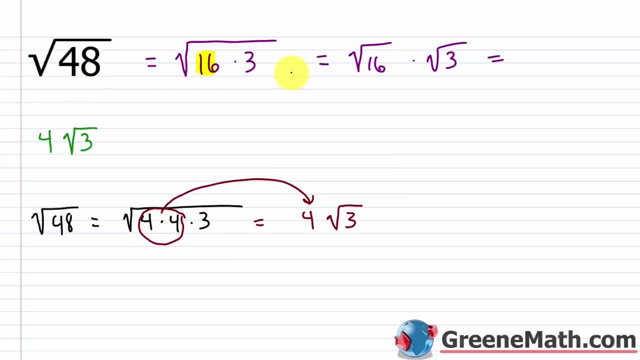 So kind of. either way you want to look at this, you're going to get the same answer. What about the square root of 12?? Well, 12,. again, I can break that down into the square root of 4 times 3.. 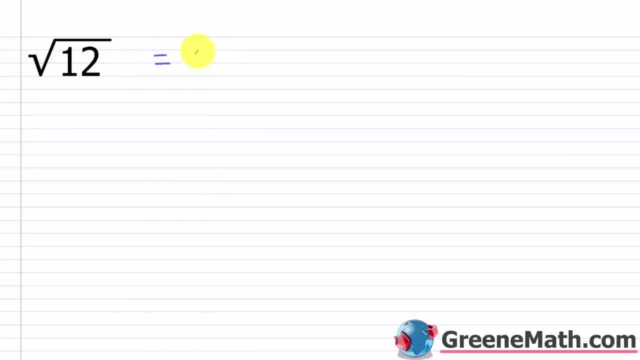 The square root of 4 is 2.. So this would be equal to the square root I'm going to do of 4 times 3.. And then I'll write the square root of 4 times the square root of 3. Again. 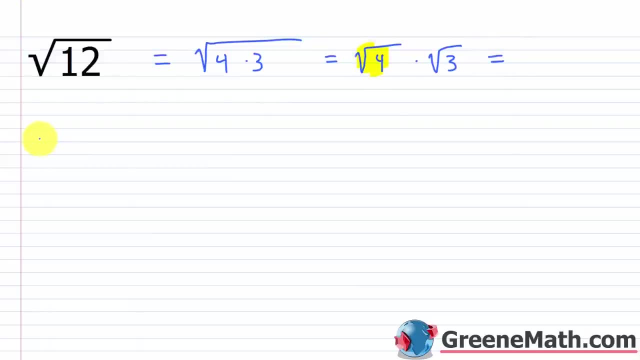 the square root of 4 is 2.. So I can just simply write that: So this would be 2 times the square root of 3.. And again, if you wanted to, you could simply say: okay, well, the square root of 12,. 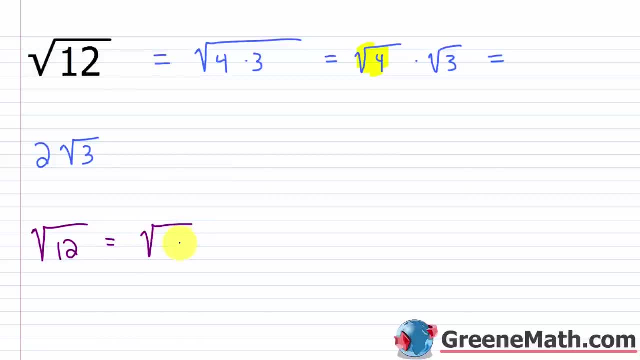 the square root of 12 is equal to the square root of 2 times 2 times 3.. So I have a pair of 2s. Okay, let me circle that. So a pair of 2s. So one of those is going to come out. 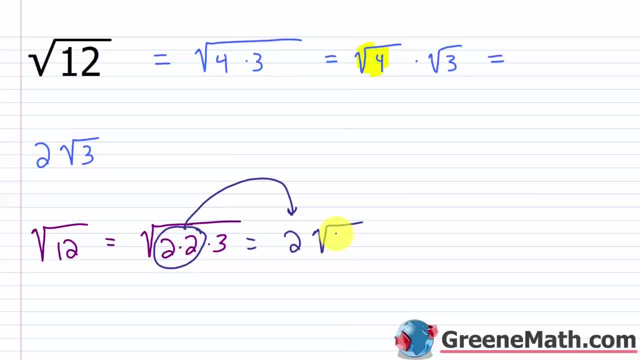 in front of the square root symbol And what's left inside is that 3.. So 2 times the square root of 3 times 3.. And then I'm going to write that down. So I have a pair of 2s And I'm going to. 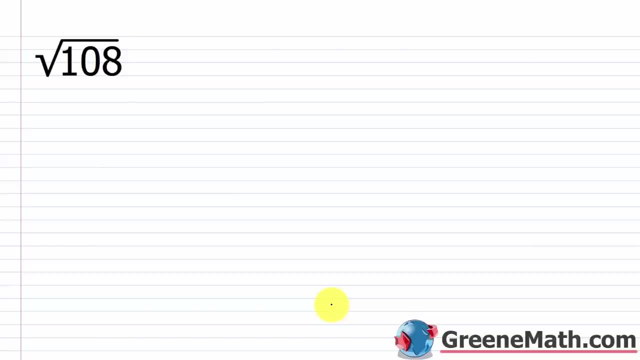 of three, kind of. either way, you do this All right. so let's take a look at one more problem before we move on and talk about the quotient rule for radicals, which again is kind of the same thing. So we have the square root of 108.. So, again, if I don't know anything about 108,- 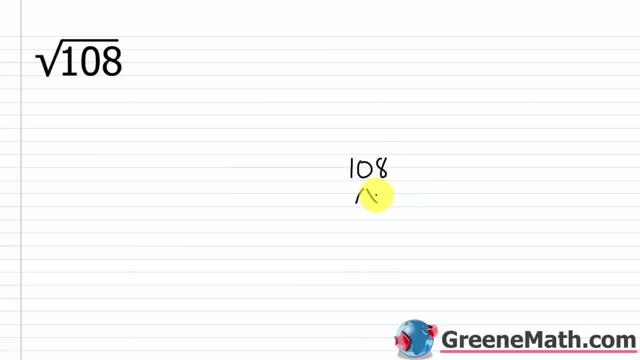 some of you might know it's prime factorization off the top of your head, others don't, right. So if I look at it, I know it's divisible by two. I know it's also divisible by four. It's what? 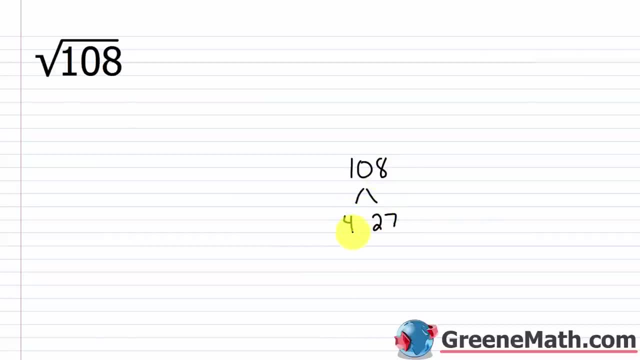 four times 27.. So I could put four times 27.. I already know that four is a perfect square, So there's something that can be pulled out here. And four I can just factor into two times two, And 27,, I know, is nine times three, So nine is another perfect square. 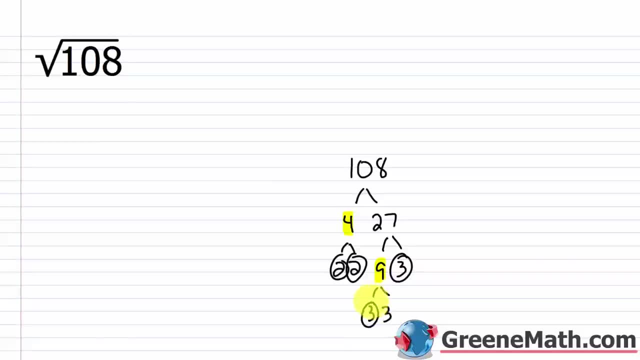 And three is prime, and then nine is three times three. Okay, so once I've kind of done that, I can eyeball this at this point and say: okay, well, I know that four is a perfect square, So two would come out. Nine is a perfect square. So 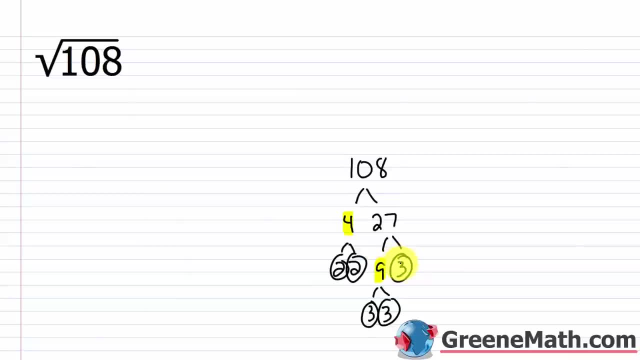 three would come out. Two times three is six. So what I'd have here is six times the square of nine. So I'd have six times the square of nine. So I'd have six times the square of nine. And I did that just from a factor tree, And you're going to get that good at it as well. 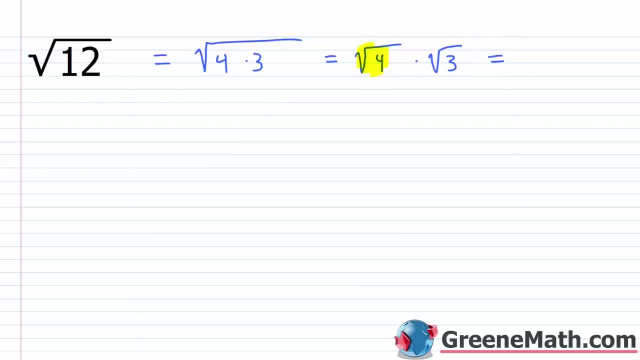 Again, we know that the square root of four is two. So I can just simply write that. So this would be two times the square root of three. 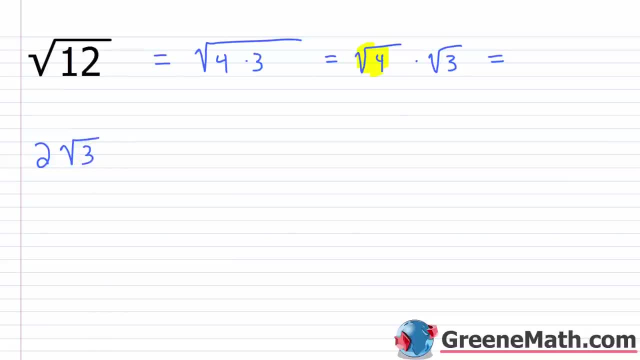 And again, if you wanted to, you could simply say, okay, well, 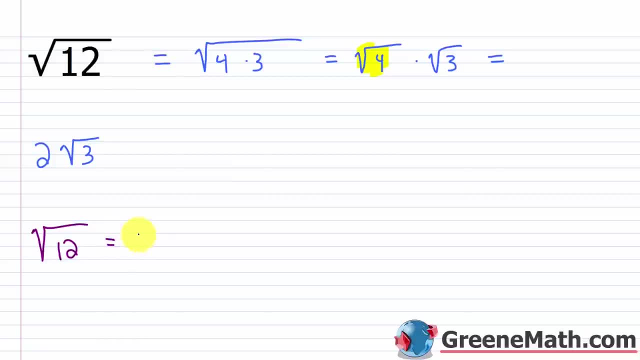 the square root of 12, the square root of 12 is equal to the square root of two times two times three. So I have a pair of twos. Okay, let me circle that. 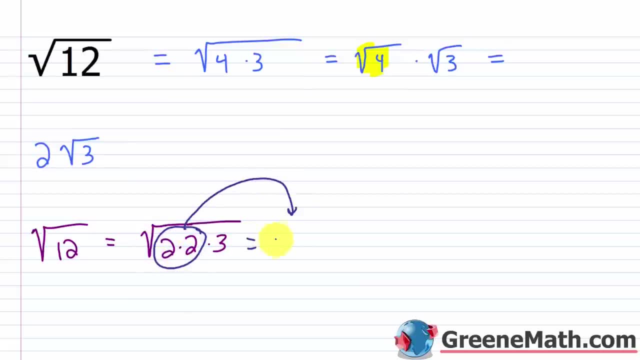 So a pair of twos. So one of those is gonna come out in front of the square root symbol. And what's left inside is that three. 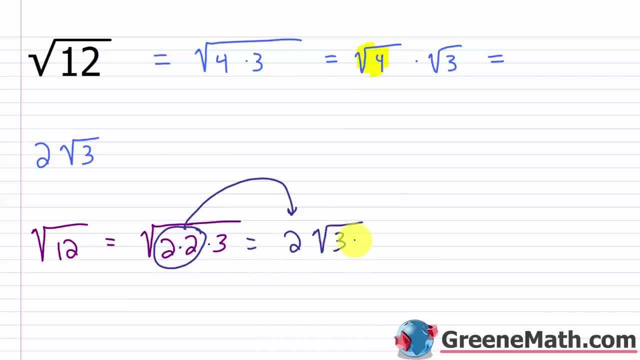 So two times the square root of three, kind of either way you do this. 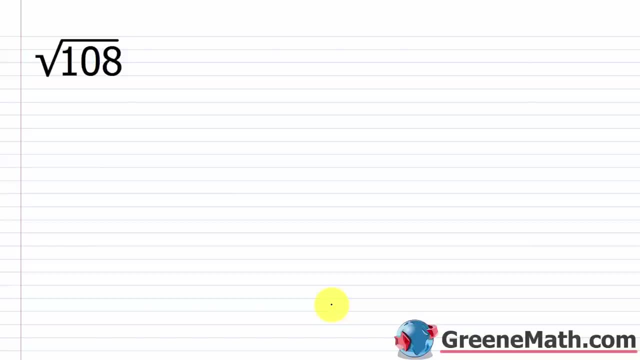 All right, so let's take a look at one more problem before we move on and talk about the quotient rule for radicals, which again is kind of the same thing. 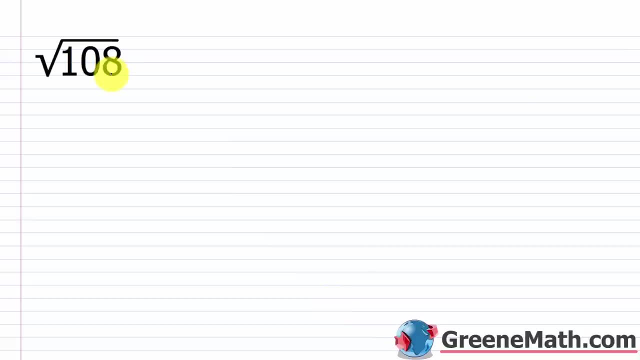 So we have the square root of 108. So again, if I don't know anything about 108, some of you might know it's prime factorization off the top of your head, others don't, right? So if I look at it, I know it's divisible by two. I know it's also divisible by four. It's what, four times 27. So I could put four times 27. I already know that four is a prime factorization. 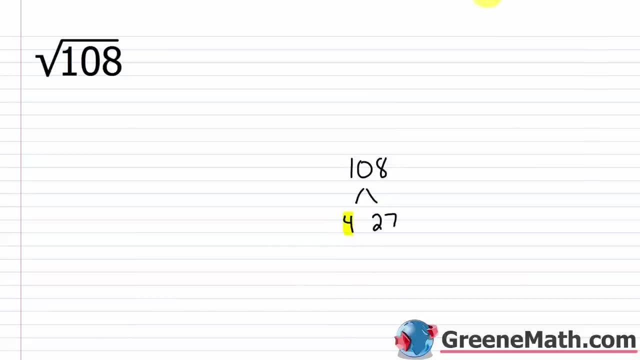 Nine is a perfect square. So there's something that can be pulled out here. And four, I can just factor into two times two. 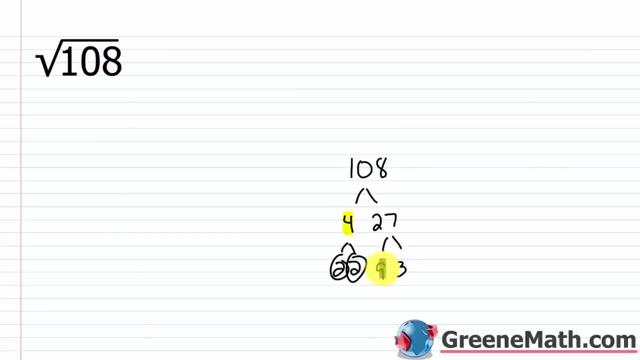 And 27, I know is nine times three. So nine is another perfect square. And three is prime, and then nine is three times three. 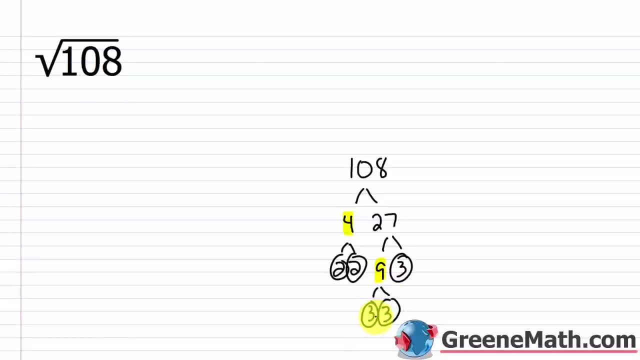 Okay, so once I've kind of done that, I can eyeball this at this point and say, okay, well, I know that four is a perfect square. 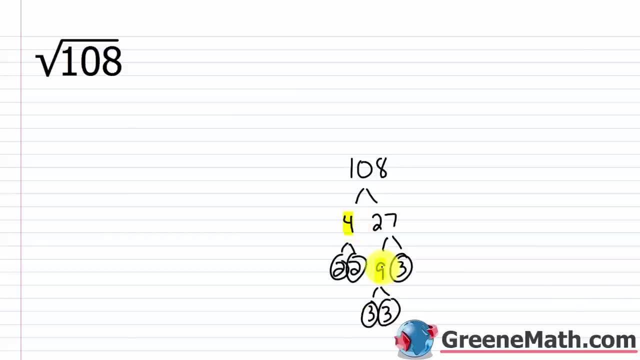 So two would come out. Nine's a perfect square, so three would come out. Two times three is six. So what I'd have here is six times the square root of three. Right, and I did that just from a factor tree. And you're gonna get that good at it as well. But for right now, let's kind of take it slow and say this is the square root of, let's do four times nine times three. 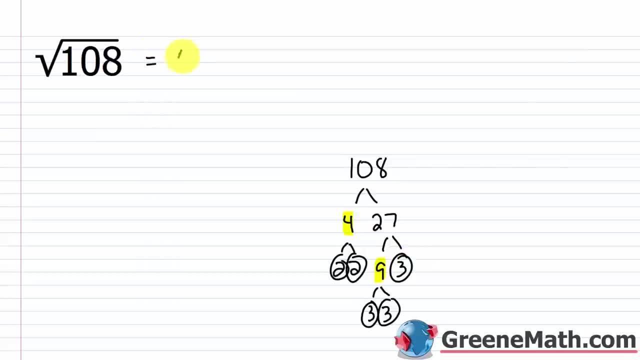 But for right now let's kind of take it slow and say: this is the square root of. let's do four times nine times three, Then we'll break this up into the square root of four times the square root of nine times the square root of three, And then we can break this up. 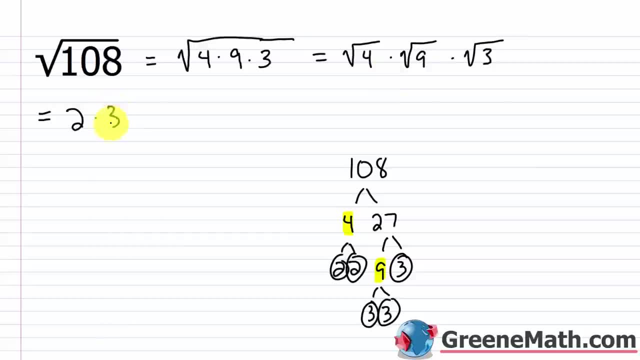 into what Square root of four is two times square root of nine is three times square root of three, And then one more time we have two times three, of that six times the square root of three, And again, this can't be simplified any further because three is a prime number. I can't break that down anymore And it's. 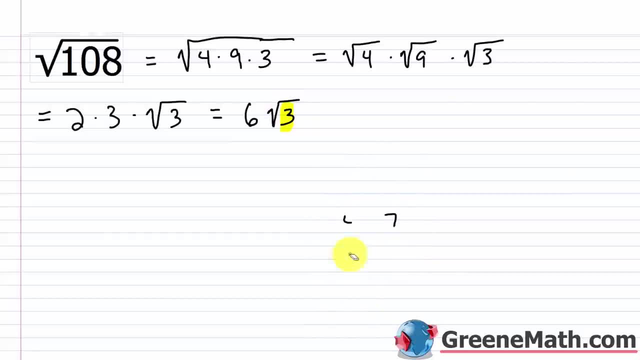 not a perfect square. So let me erase this. And one last time. let me just show you the alternative way to do it. So if I have the square root of 108, this is equal to what The square root of. let's do two times two times three times, three times three. So then again for each pair. 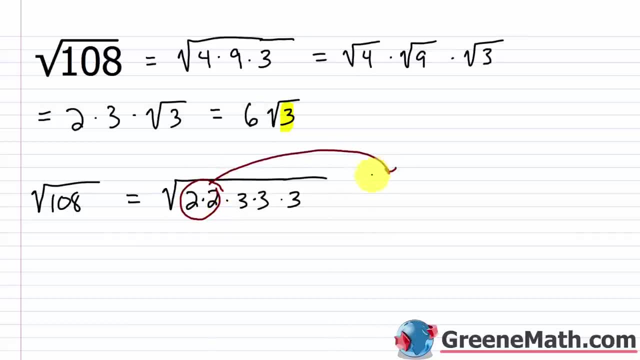 I'm going to pull one out. So this is a pair. So I'm going to pull that out. This is a pair. I'm going to pull that out and then nothing to really pair with that. So let me not circle it, Let me put. 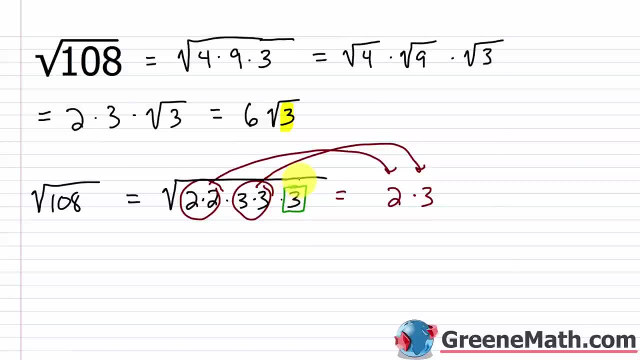 a little box around it so we can identify that it's different. So we'll put the square root of three for that. So this equals two times three is six And again times the square root of three. So again, either way you do it, you're going to get six times the square root of three. 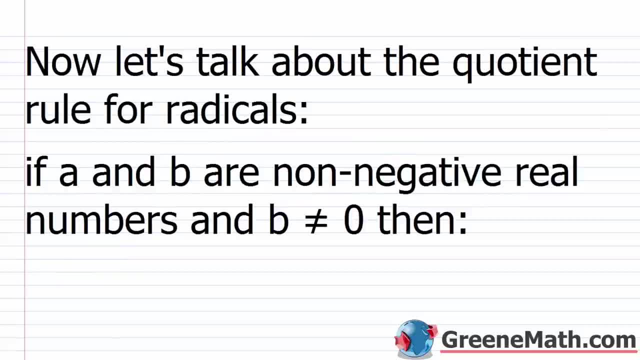 So overall it's not too difficult to simplify radicals Once you kind of understand the basics and you have a general idea of what's going on. it's just basic arithmetic. So now we want to talk about the quotient rule. for radicals, This is no more difficult, particularly in algebra one. 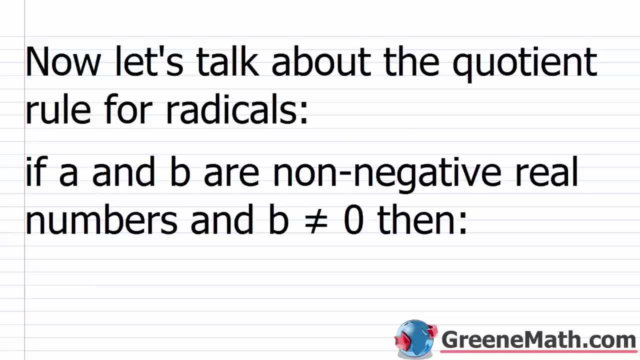 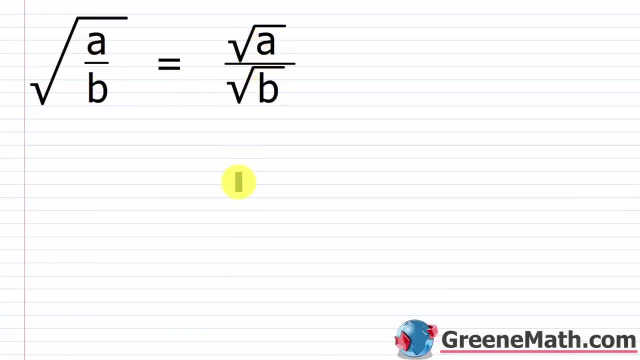 they're not going to give you anything. that's too challenging, And we're just going to start by saying: if A and B are non-negative- again non-negative- real numbers and B is not equal to zero, then we have this of: A over B is equal to the square root of A over the square root of B. So all we're doing is we're. 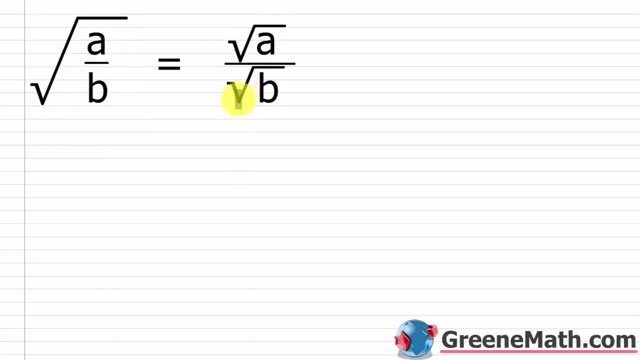 separating this into the numerator having a square root and the denominator having a square root. So, in other words, if I had something like the square root of one fourth, we know at this point this is equal to one half, but we can break it down and say the square root of one fourth. 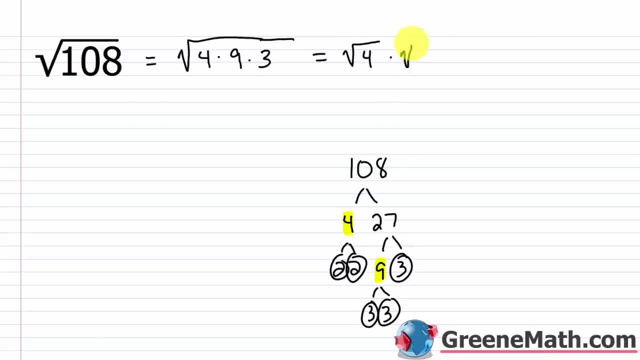 Then we'll break this up into the square root of four times the square root of nine times the square root of three. 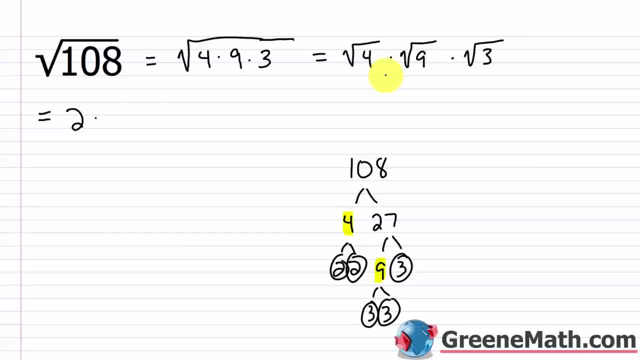 And then we can break this up into what? Square root of four is two times square root of nine is three times square root of three. 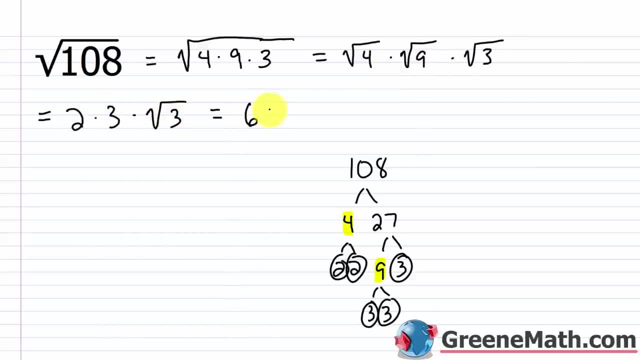 And then one more time, we have two times three, that's six times the square root of three. 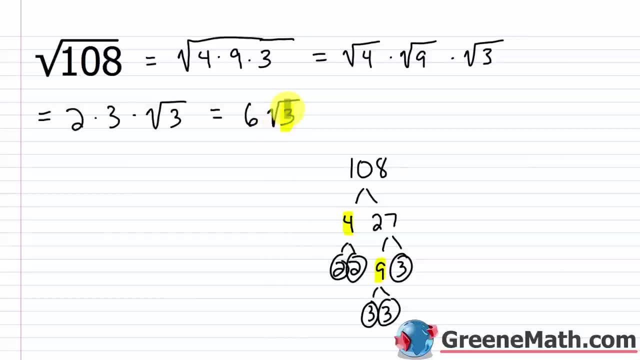 And again, this can't be simplified any further because three is a prime number. I can't break that down anymore. And it's not a perfect square. So let me erase this. And one last time, let me just show you the alternative way to do it. 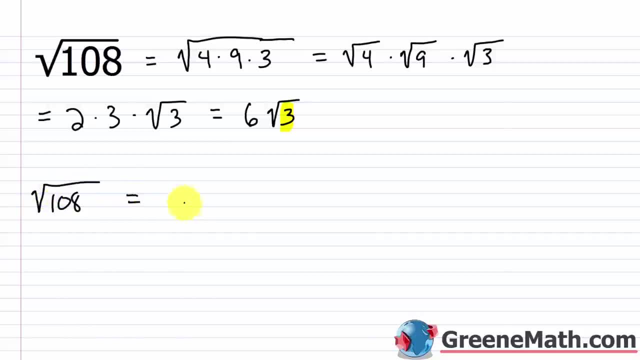 So if I had the square root of 108, this is equal to what? The square root of, let's do two times two times three times three times three. And for each pair, I'm gonna pull one out. 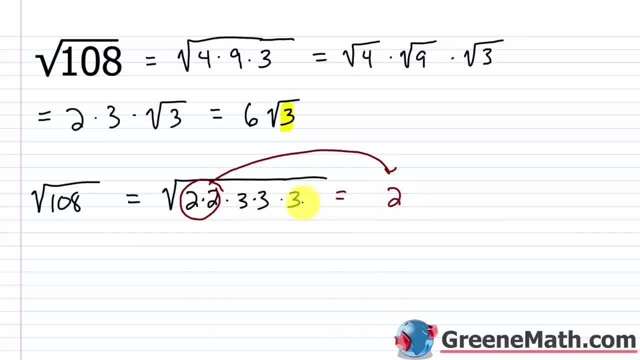 So this is a pair. So I'm gonna pull that out. This is a pair, I'm gonna pull that out. 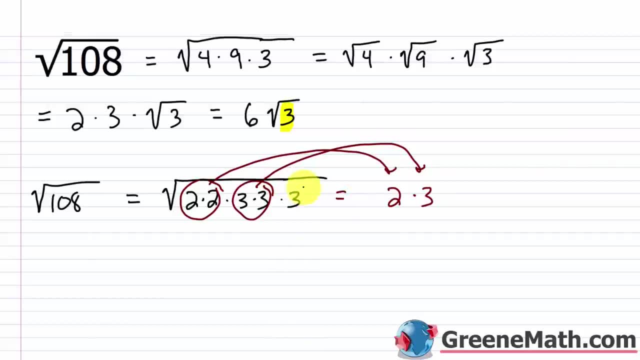 And then nothing to really pair with that. So let me not circle it. Let me put a little box around it so we can identify that it's different. So we'll put the square root of three for that. So this equals two times three is six. 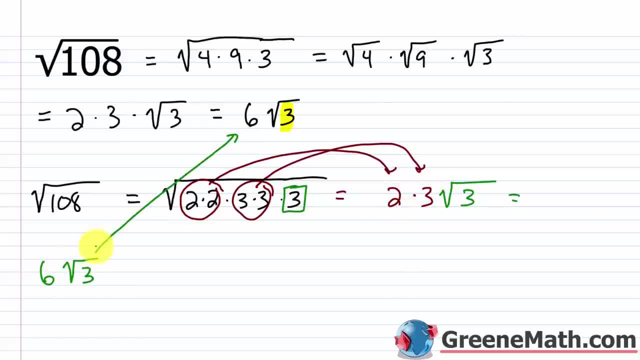 And again, times the square root of three. So again, either way you do it, you're gonna get six times the square root of three. 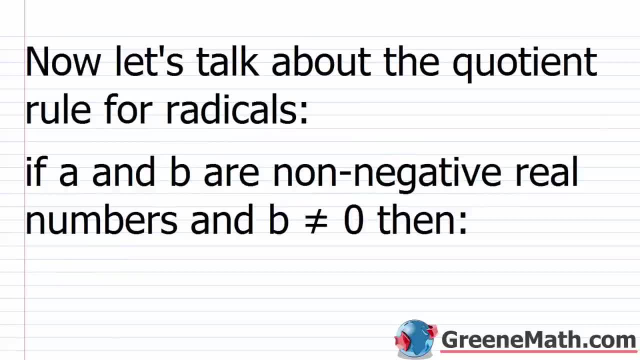 So overall, it's not too difficult to simplify radicals. Once you kind of understand the basics and you have a general idea of what's going on, it's just basic arithmetic. 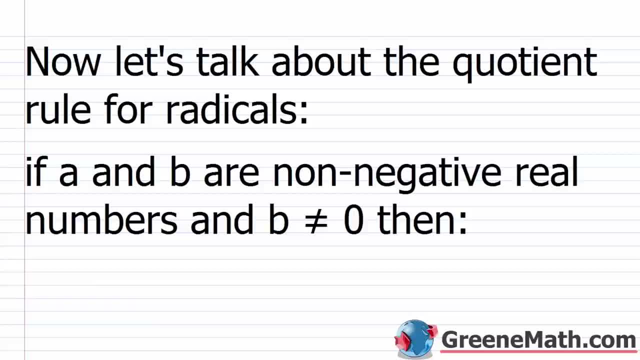 So now we wanna talk about the quotient rule for radicals. This is no more difficult, particularly in algebra one, they're not gonna give you anything that's too challenging. 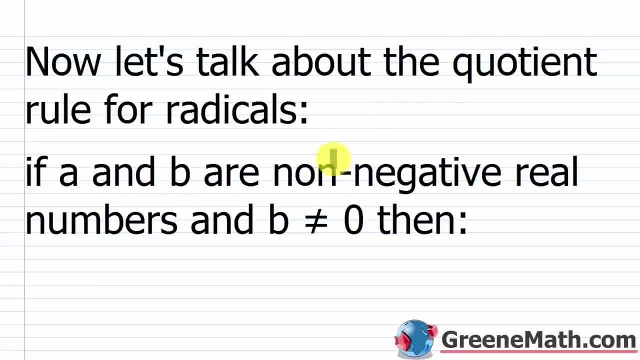 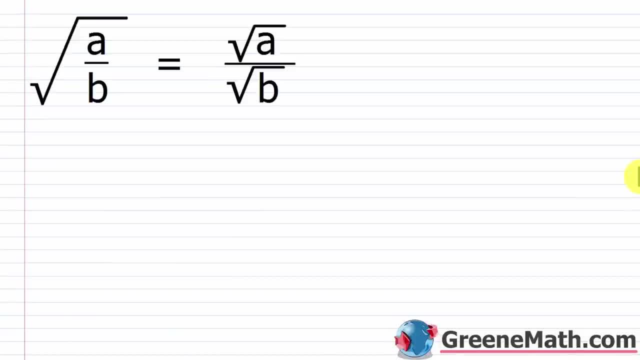 And we're just gonna start by saying, if A and B are non-negative, again, non-negative, real numbers, and B is not equal to zero, then we have this. The square root of A over B 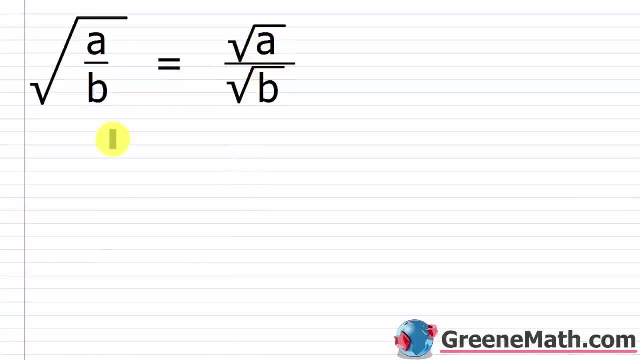 is equal to the square root of A over the square root of B. So all we're doing is we're separating this into the numerator having a square root and the denominator having a square root. So in other words, 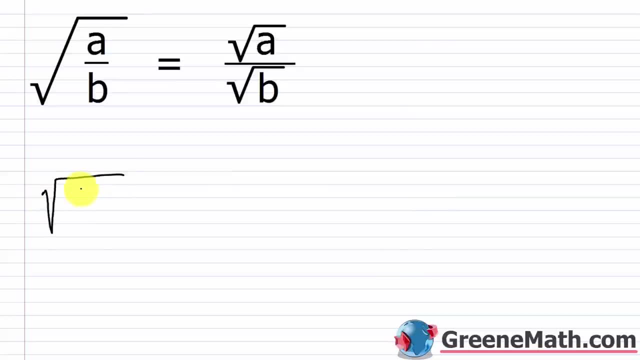 if I had something like the square root of 1 4th, we know at this point, this is equal to 1 1⁄2, but we can break it down and say the square root of 1 4th is equal to the square root of one over the square root of four so this is equal to what? Square root of one is one, square root of four is two. 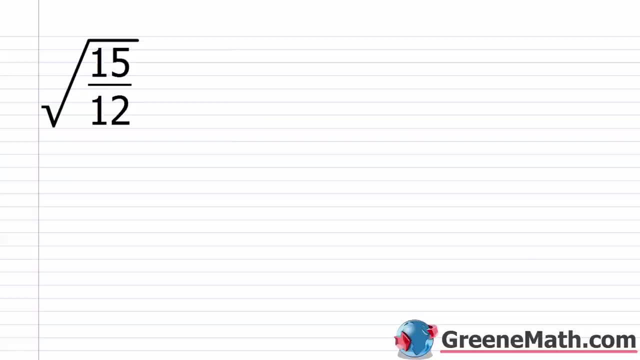 So we can see that that is mathematically valid. All right, so what about something like 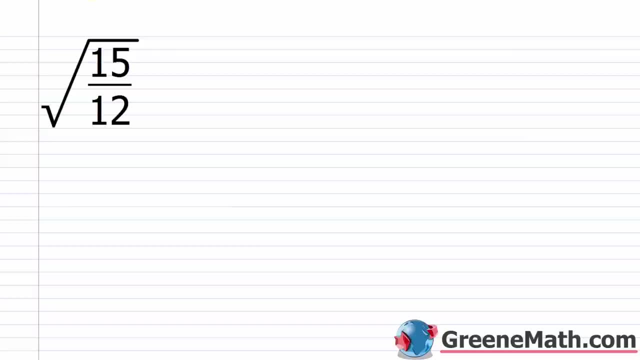 the square root of 15 over 12? Well, when you get a problem like this, what they want you to do is just go through the steps. And in most cases, they're gonna give you a bunch of stuff that's going to cancel out so you can simplify. So this would be the square root of 15 over the square root of 12. But don't just do that. 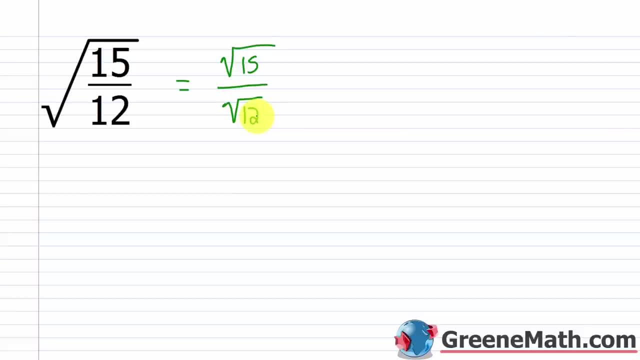 Once you've separated it, look for the square root of 12. So don't just do that. Look for ways to simplify it 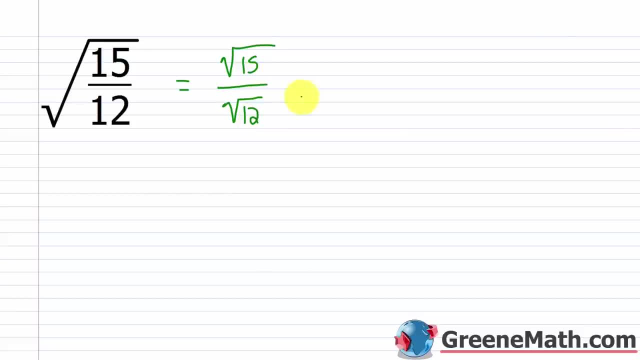 based on what you did in the previous section. So I know the square root of 15 is what? 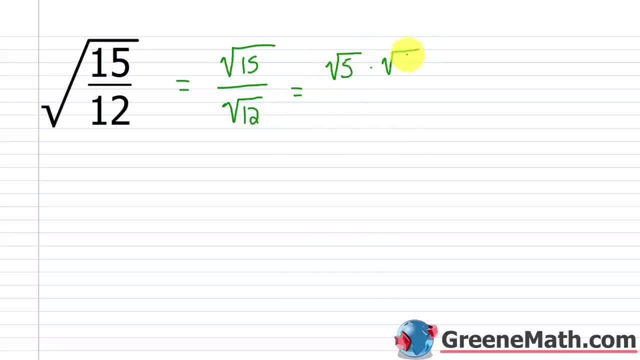 It's the square root of five times the square root of three. Okay, I can't do anything with either of those, but if you look at the square root of 12, I know I can break that up into what? I know I can do the square root of four times the square root of three. 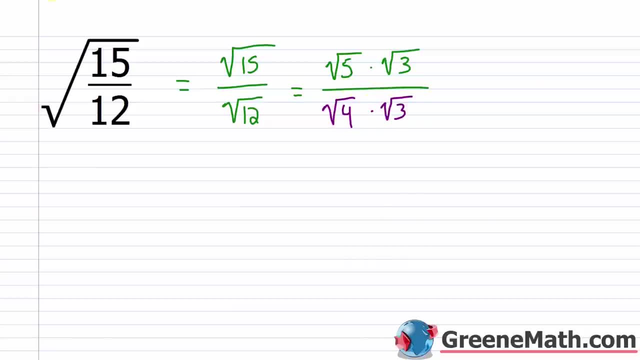 Now, square root of three over square root of three is what? If I gave you the square root of three over the square root of 12, I'd give you the square root of three. This is the same non-zero number over itself. So this is going to cancel and be equal to one, okay? 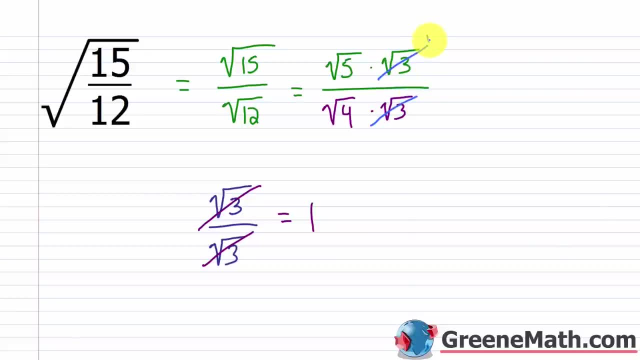 So these same rules apply. So this cancels with this, that's a one. So now what I'm left with is the square root of five, which I can't do anything with, over the square root of four, which we know is two. 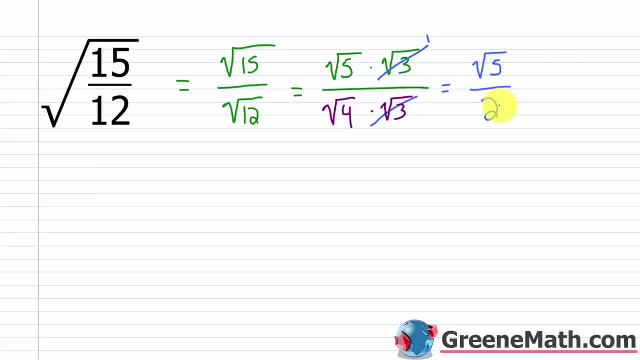 So I end up with the square root of five over two for my simplified answer. All right, let's take a look at another one. 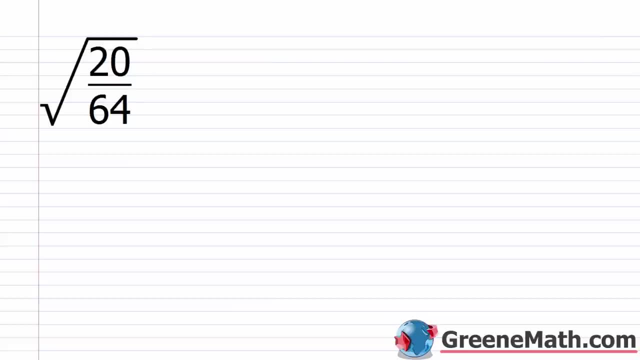 Let's say we have the square root of 20 over 64. All right, so again, what we're meant to do here is just break this up into the square root of 20 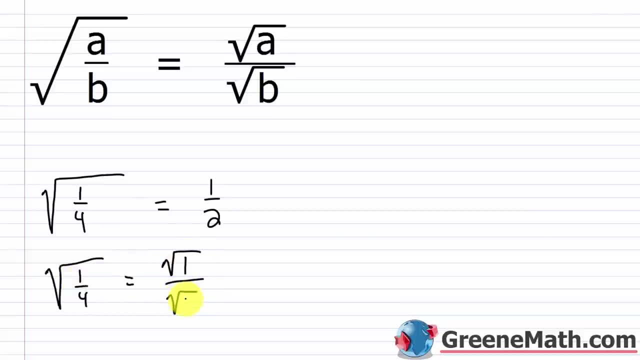 is equal to the square root of one over the square root of four. So it's equal to what Square root of one is one. square root of four is two. So we can see that that is mathematically valid. All right. so what about something like the square root of 15 over 12?? Well, when you get a 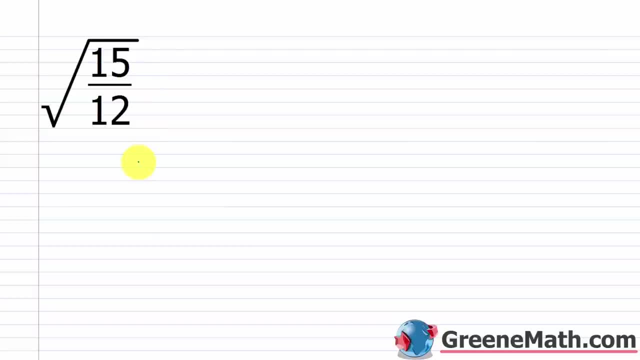 problem like this. what they want you to do is just go through the steps And in most cases they're going to give you a bunch of stuff that's going to cancel out. so you can simplify. So this would be the square root of 15 over the square root of 12.. But don't just do that Once you've. 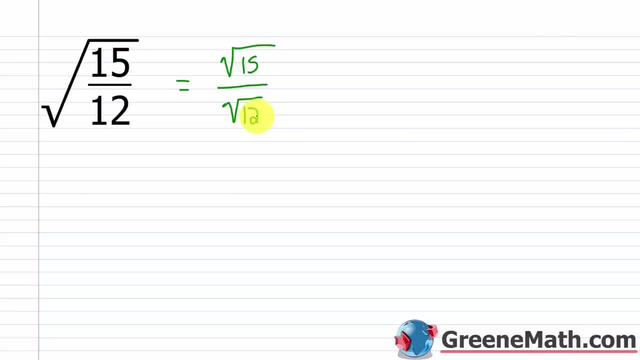 separated it. look for ways in which you can simplify it. So let's say you have a square root of five over 12.. What you can do is simplify it based on what you did in the previous section. So I know the square root of 15 is what It's: the square root of five times the square root of three. 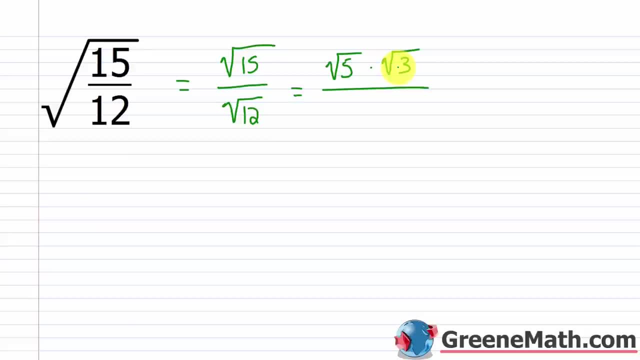 Okay, I can't do anything with either of those. But if you look at the square root of 12, I know I can break that up into one. I know I can do the square root of four times the square root of three. Now, square root of three over square root of three is one. 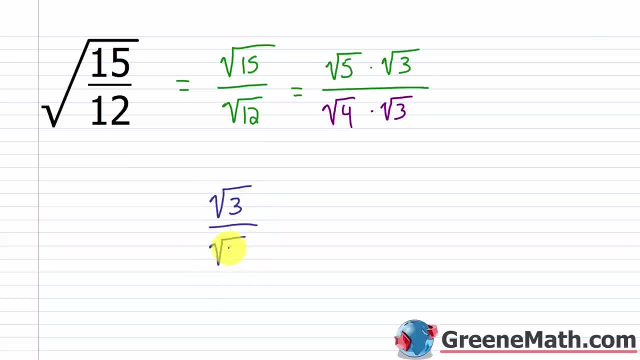 If I gave you the square root of three over the square root of three, the same non-zero number over itself. so this is going to cancel and be equal to 1,. okay, So these same rules apply. So this cancels with this. that's a 1.. So now what I'm left with is the square root. 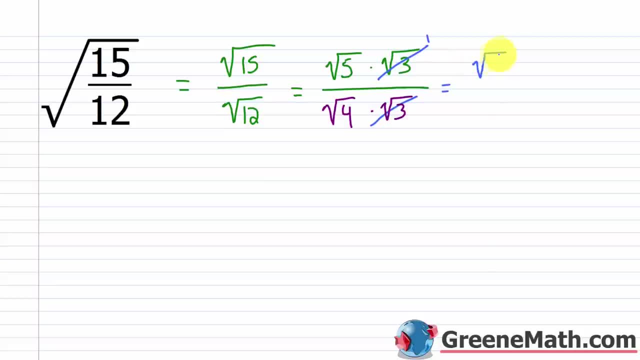 of 5,, which I can't do anything with, over the square root of 4, which we know is 2.. So I end up with the square root of 5 over 2 for my simplified answer. All right, let's take a look at another. 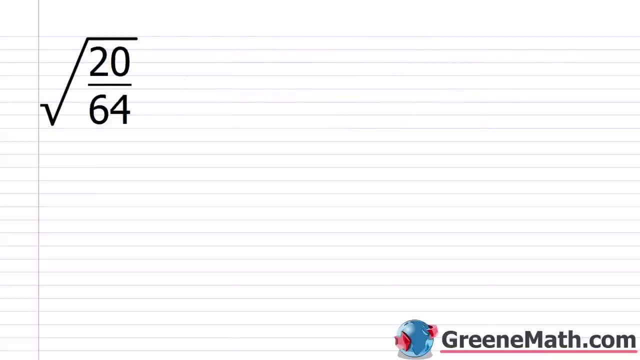 example, Let's say we have the square root of 20 over 64.. All right, so again, what we're meant to do here is just break this up into the square root of 20 over the square root of 64.. Now, 64 is a. 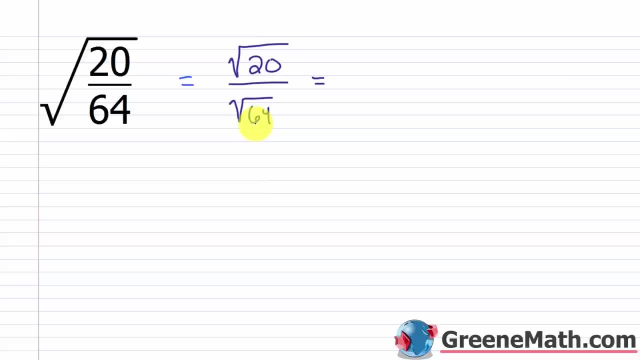 perfect square. so all I really need to do in that is just take the square root and that's going to be 8.. That's simple enough. Now for the square root of 20, I could break that up as the square. over the square root of 64. 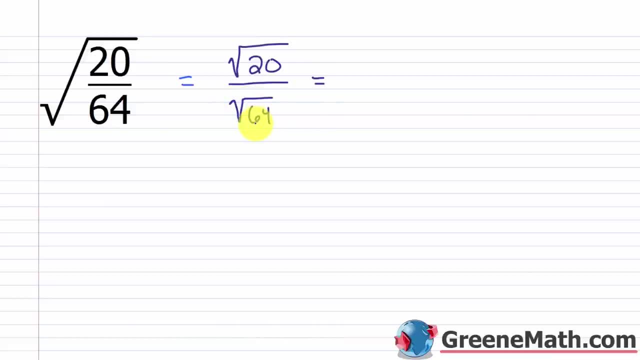 Now, 64 is a perfect square. So all I really need to do in that is just take the square root and that's going to be eight. That's simple enough. Now for the square root of 20, 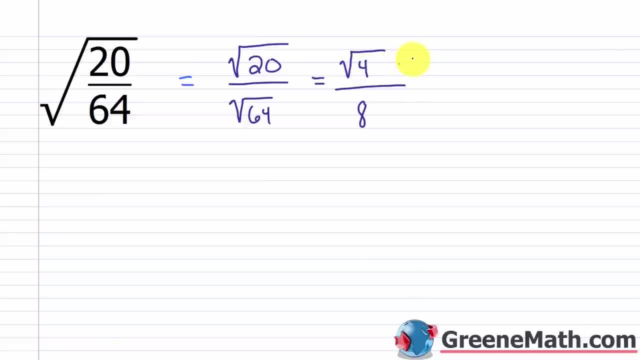 I could break that up as the square root of four times the square root of five. I know the square root of four is two, so I could just write this in. 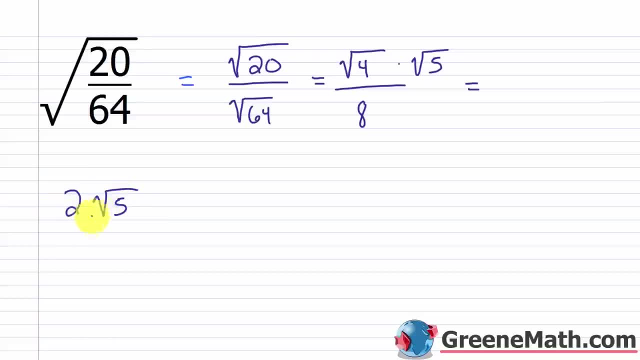 I could write this as two times square root of five over eight. So because this is straight multiplication, I can cancel common factors. 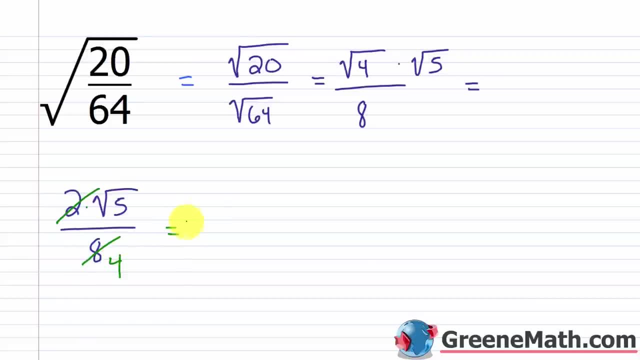 So this two would cancel with this eight and give me a four. So this would simply be the square root of five over four. 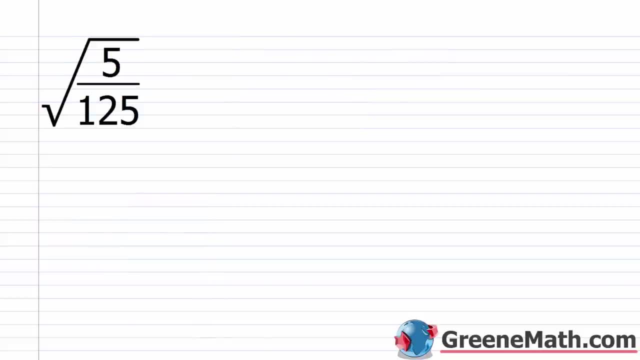 All right, so for the next one, we can kind of simplify this two different ways. Kind of the way we've been doing it so far, we could set this up as what? 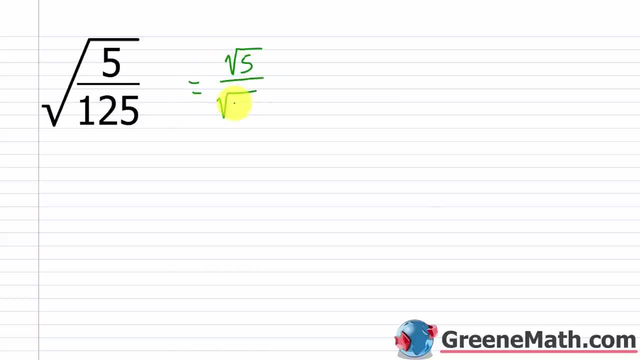 The square root of five over the square root of 125. 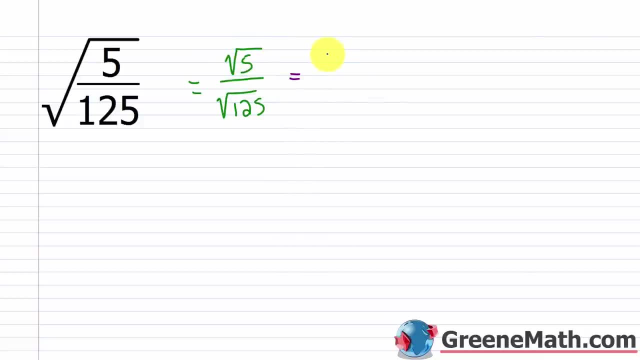 Obviously, I can't do anything with the square root of five, but what I can do is something with the square root of 125. 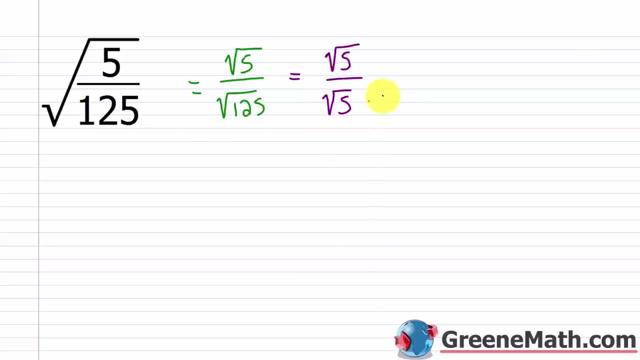 I can write this as the square root of five times the square root of 25. Now we already know that this will cancel with this, right? 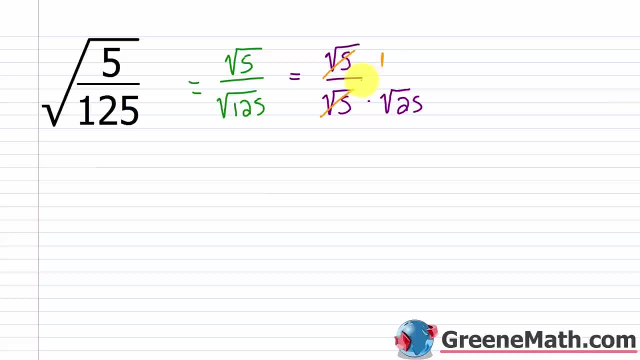 Square root of five over square root of five is one. So I'm going to write a one for the numerator there. And then the square root of 25 is five. So let me just write that this is equal to one over five. 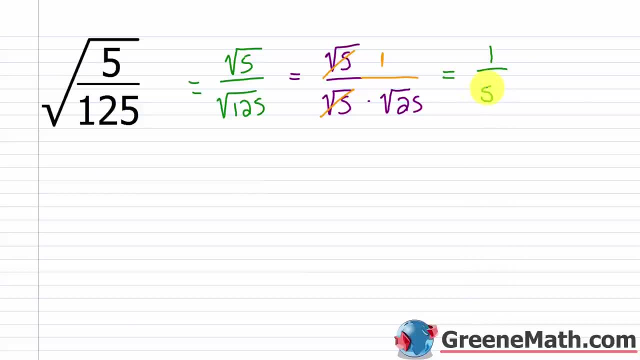 Now, in this particular situation, I could have gotten that by just simplifying the fraction to start, right? If I divide 125 by five, I get 25. 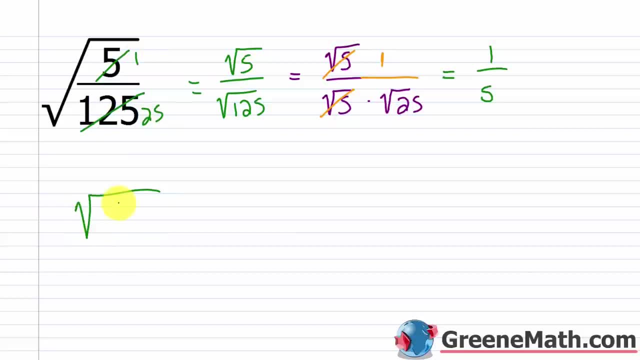 If I divide five by five, I get one. So if I had the square root of one over 25, basically, if I think about that in my head, the square root of one is one, and the square root of 25 is five. So that's kind of a quicker way to do that in this scenario. And you get the same answer either way. 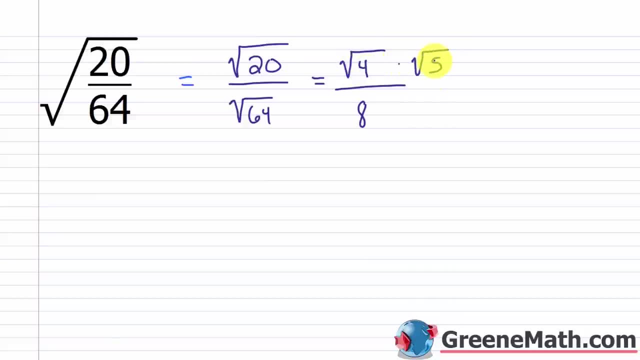 root of 4 times the square root of 5.. I know the square root of 4 is 2, so I could just write this as 2 times square root of 5 over 8.. So because this is straight multiplication, I can cancel common factors. So this 2 would cancel with this 8 and give me a 4.. 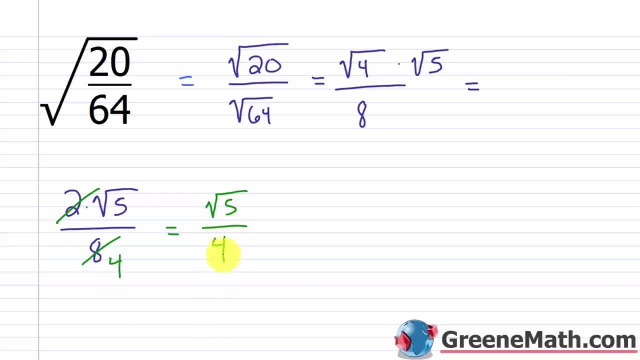 So this would simply be the square root of 5 over 4.. All right, so for the next one, we can kind of simplify this two different ways, Kind of the way we've been doing it so far. we could set this up. 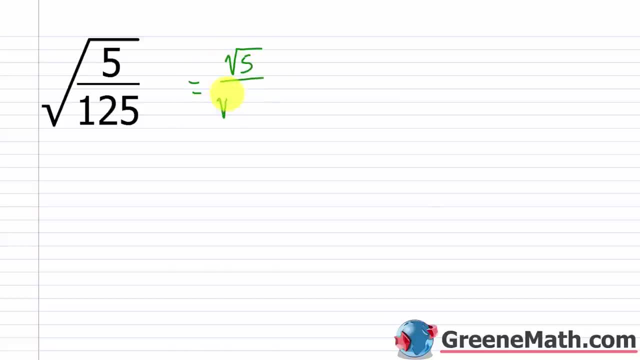 as what? The square root of 5 over the square root of 125.. Obviously, I can't do anything with the square root of 5, but what I can do is something with the square root of 125. I can write this as the square root of 5 times the square root of 25.. Now we already know. 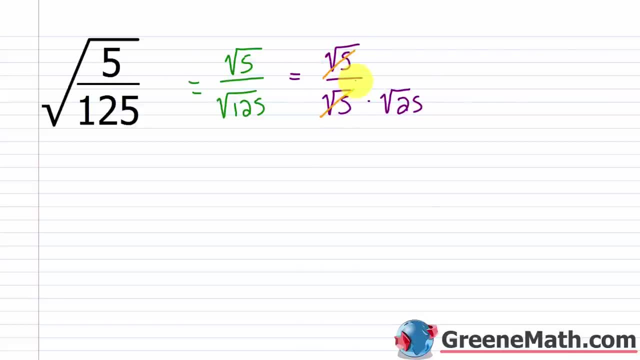 that this will cancel with this right Square root of 5 over. square root of 5 is 1.. So I'm going to write a 1 for the numerator there, and then the square root of 25 is 5.. So let me just write: 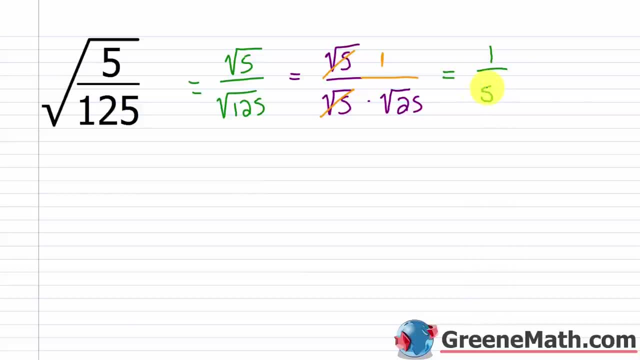 that this is equal to 1 over 5.. Now, in this particular situation, I could have gotten that by just simplifying the fraction. to start right, If I divide 125 by 5, I get 25.. If I divide 5 by 5, I get 1.. So if I have the square root of 1, 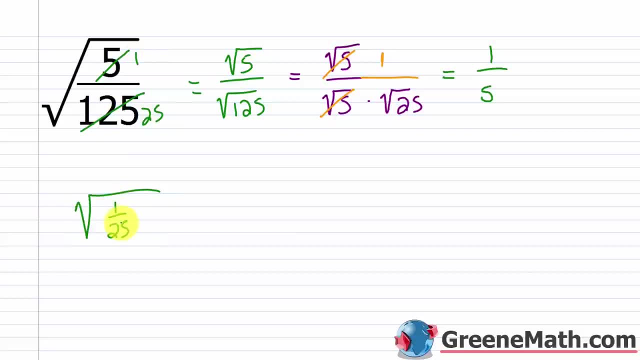 over 25,. basically, if I think about that in my head, the square root of 1 is 1, and the square root of 25 is 5.. So that's kind of a quicker way to do that in this scenario and you get the same. 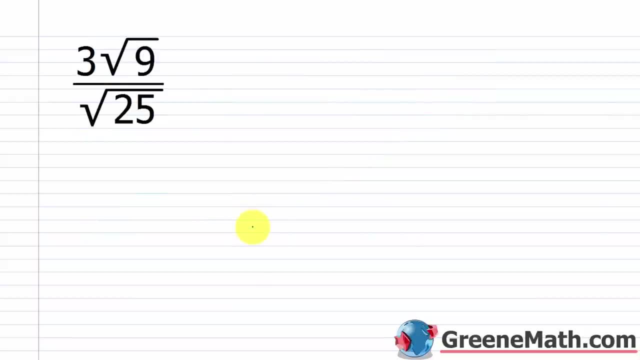 answer either way. What about something like 3 times the square root of 9 over the square root of 25?? We know the square root of 9 is 3, so this would be 3 times 3 over the square root of 25 is 5.. 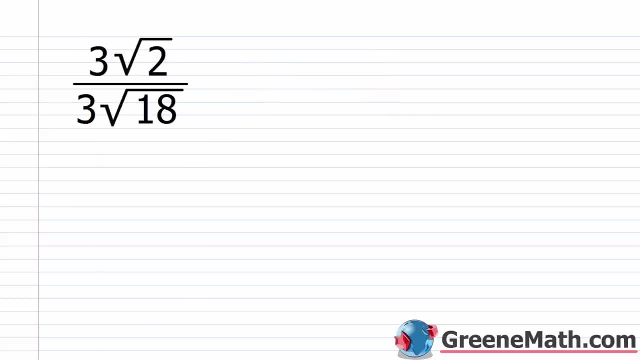 So this would be 9 fifths. What about something like 3 times the square root of 2 over 3 times the square root of 18?? Well, right away again, because this is all multiplication. we could just cancel this with this to start and just say I have the square root of 2 over the square root of. 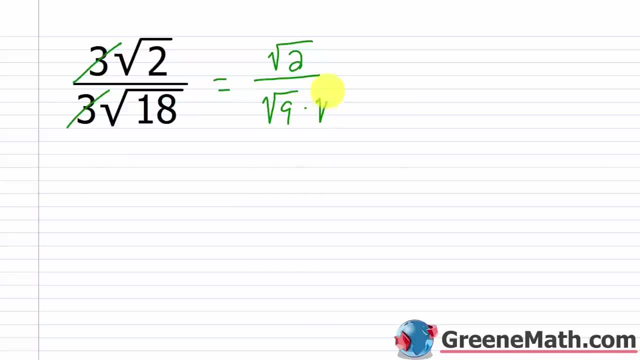 18,, which I could say is the square root of 9 times the square root of 2, and I can break this down because this is 3.. And then this would cancel with this. so what I'm left with is a 1 for my. 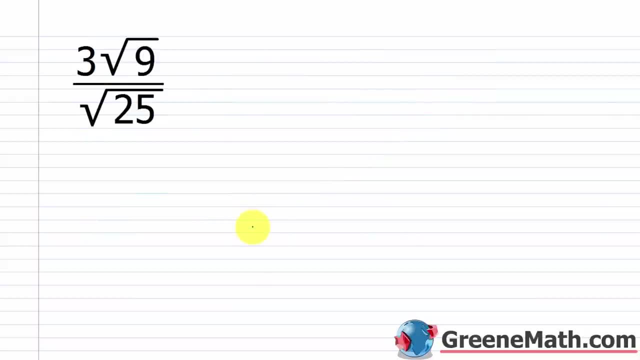 What about something like three times the square root of nine, over the square root of 25? We know the square root of nine is three, so this would be three times three, over the square root of 25 is five. So this would be nine fifths. 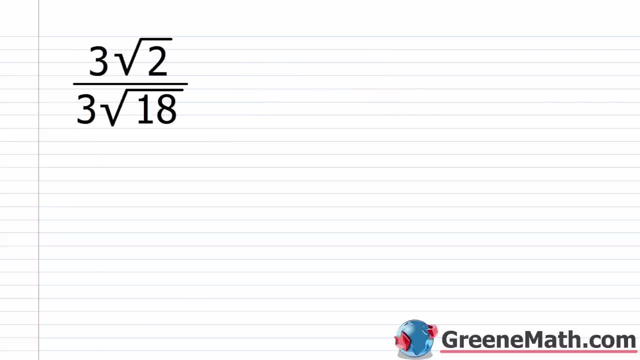 What about something like three times the square root of two, over three times the square root of 18? Well, right away, again, because this is all multiplication, we could just cancel this with this to start. And just say I have the square root of two over the square root of 18, which I could say is the square root of nine times the square root of two. 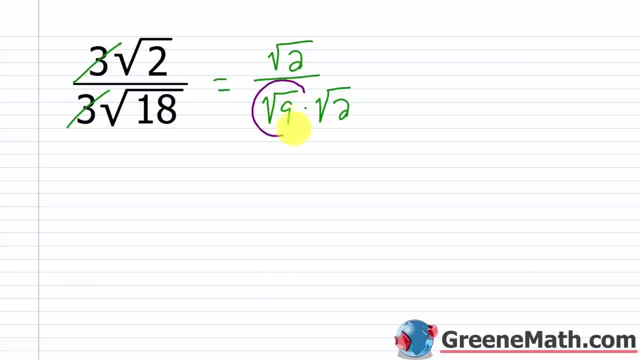 And I can break this. I can break this down further, because this is three. 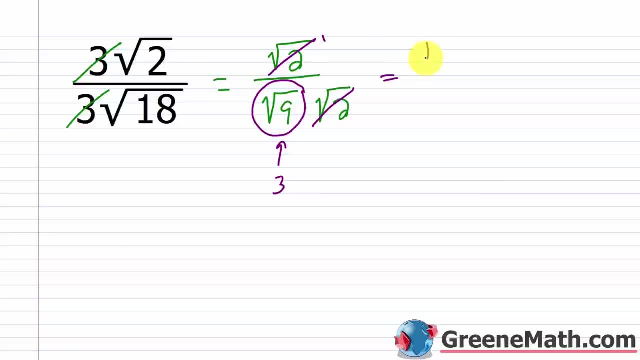 And then this would cancel with this. So what I'm left with is a one for my numerator, and then a three for my denominator. So this is gonna be equal to one third. 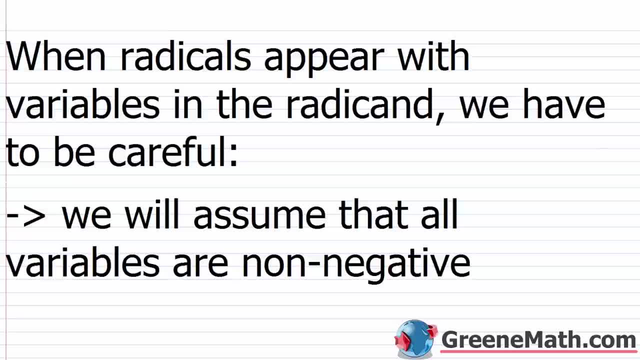 So all in all, simplifying radicals is a very, very easy topic. 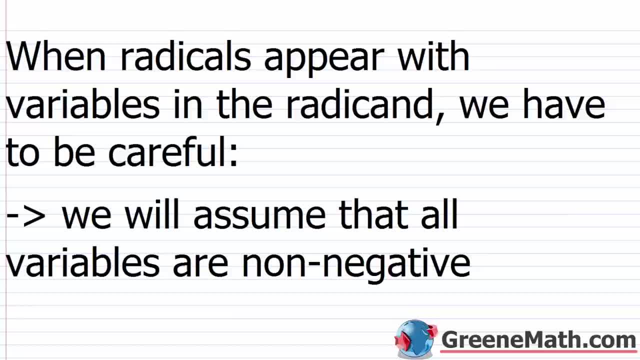 We're gonna start to get into some stuff that's a little bit more challenging now. 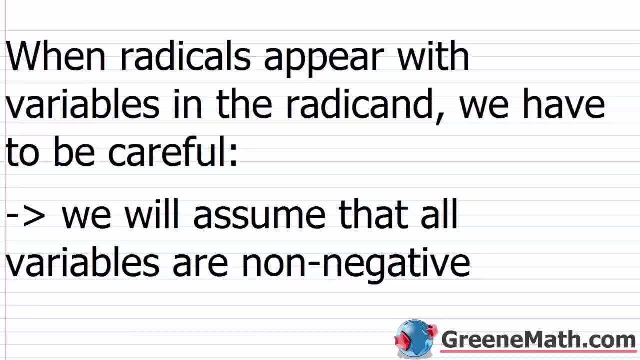 We're gonna start talking more about variables and higher level roots. 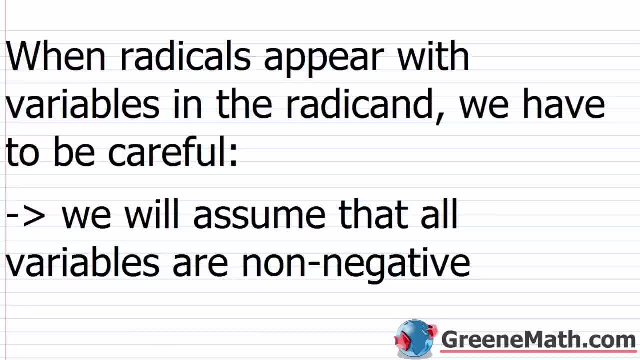 So when radicals appear with variables in the radicand, we have to be very careful. Why do we have to be careful? Why do we have all these restrictions? 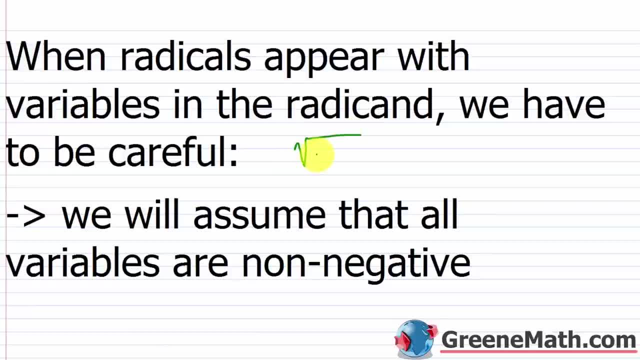 Well, I want you to remember that if you have something like the square root of, let's say, negative four, 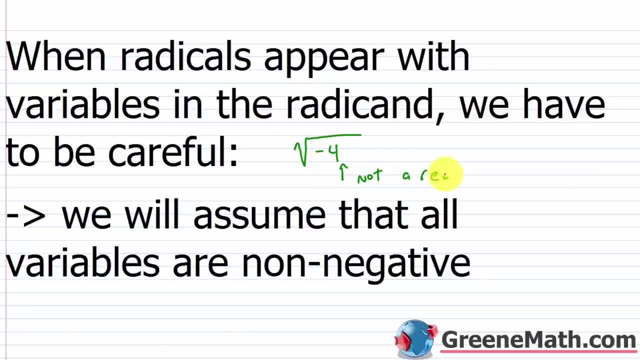 this is not a real number. 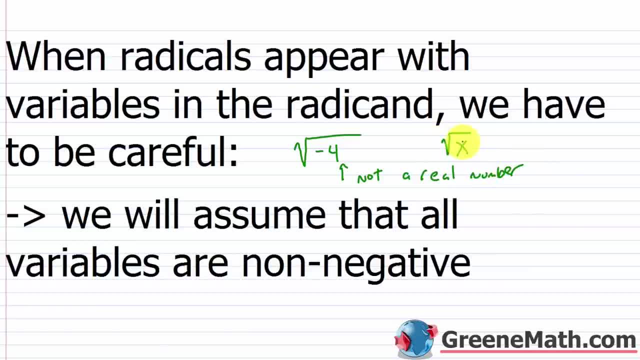 So if I gave you the square root of x, can I assign x to be negative four? No, I cannot, right? Because that's not a real number. 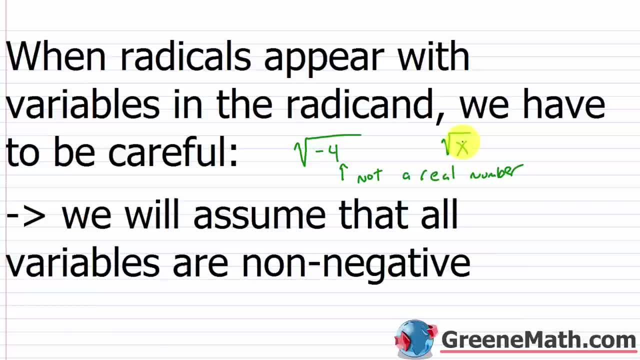 Later on, at the end of algebra one, and as we get into algebra two and college algebra, we're gonna have these things called imaginary numbers that allow us to deal with negative square roots, but we haven't gotten there yet. 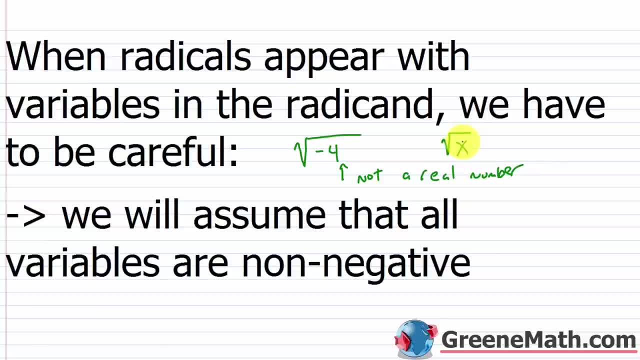 So for right now, we're just gonna say that the variables that appear in the radicand are going to be non-negative. So let's take a look at one 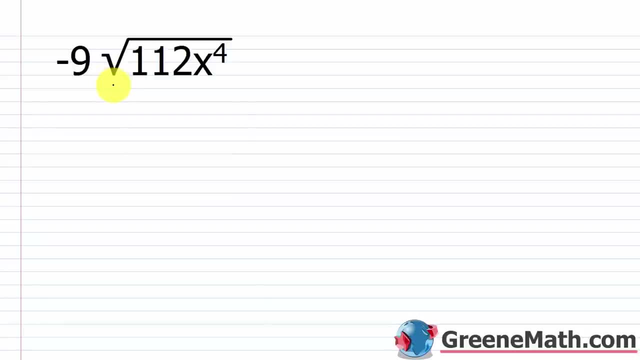 that's a little bit more challenging. So we have negative nine times the square root 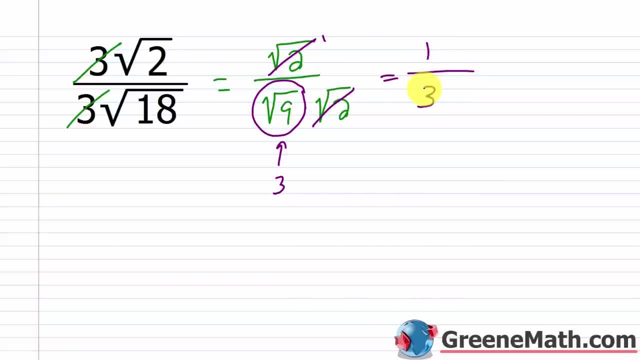 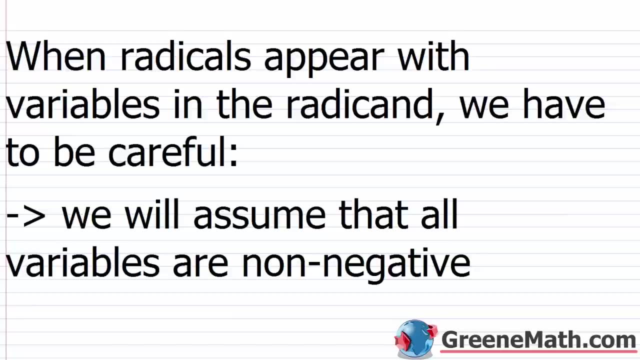 numerator and then a 3 for my denominator. so this is going to be equal to 1 third. So, all in all, simplifying radicals is a very, very easy topic. We're going to start to get into some stuff that's a little bit more challenging now. We're going to start talking more about variables and 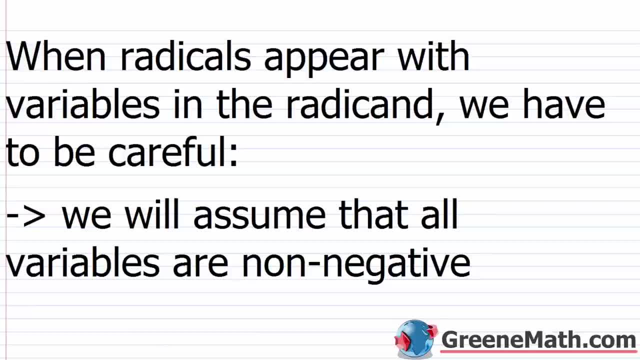 higher level roots. So when radicals appear with variables in the radicand, we have to be very careful. Why do we have to be careful? Why do we have all these restrictions? Well, I want you to remember that if you have something like the square root of, let's say, negative 4, this is not. 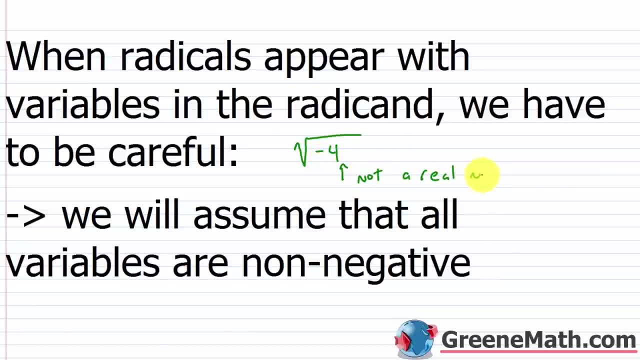 a real number. So if I gave you the square root of x, can I assign x to be negative 4?? No, I cannot right, Because that's not a real number. Later on, at the end of Algebra 1,: 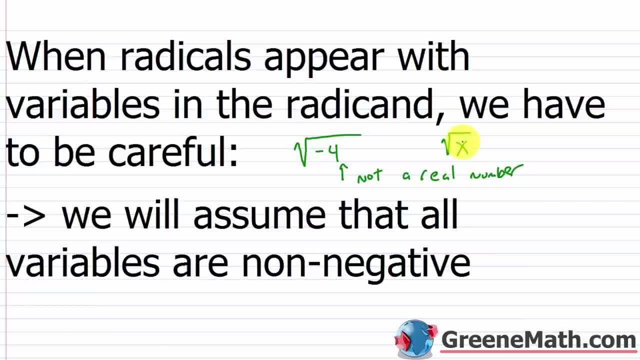 and as we get into Algebra 2 and College Algebra, we're going to have these things called imaginary numbers that allow us to deal with negative square roots. but we haven't gotten there yet, So for right now we're just going to say that the variables that appear in the radicand are going to: 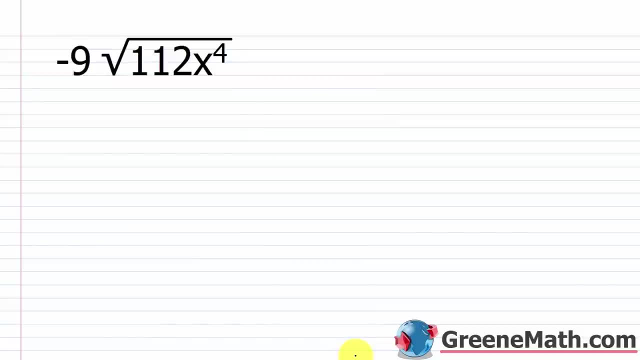 be non-negative. So let's take a look at one that's a little bit more challenging. So we have negative 9 times the square root of 112x to the fourth power. So just put your negative 9 out in front and then times the square root of. Let's try to break this down inside and let's just start. 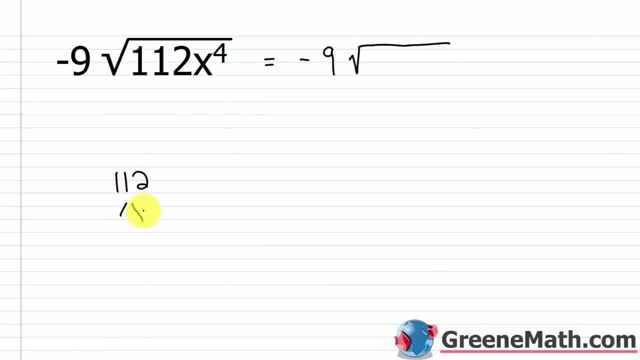 with the number part. So 112, I know- is divisible by 2.. It's also divisible by 4, right, The last two digits would be a 12. So obviously that's divisible by 4. It would be 4 times 28.. So let's start with that. 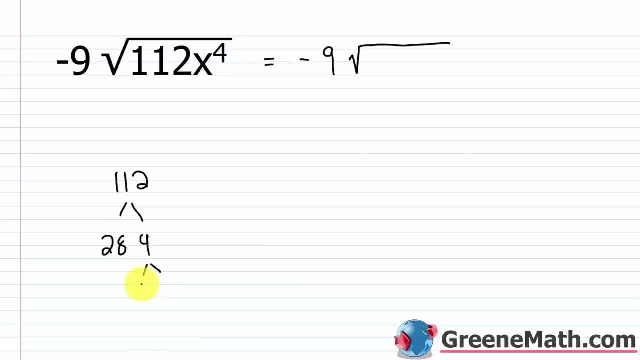 28 times 4.. 4 is a perfect square: It's 2 times 2.. 28 is 4 times 7.. Again, 4 is a perfect square: It's 2 times 2.. So at this point I know the number part. the square root of 112 would simplify. 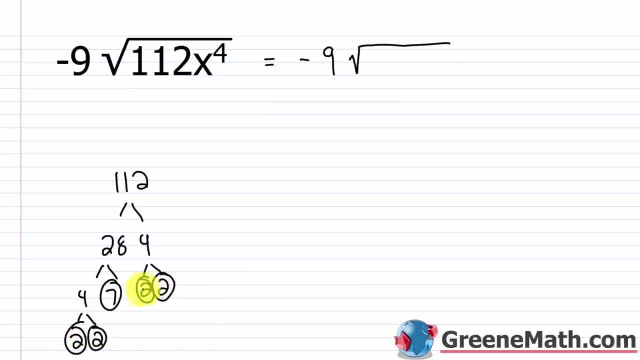 to what? 2 times 4.. 2 times 2, or 4 times the square root of 7, right? So once you start getting good at this, you can kind of eyeball that and say, okay, I would have 4 outside of the symbol, okay, And. 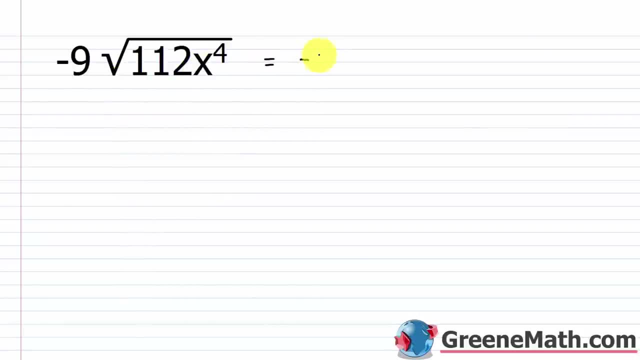 of 112x to the fourth power. So just put your negative nine out in front, and then times the square root of, let's try to break this down inside. 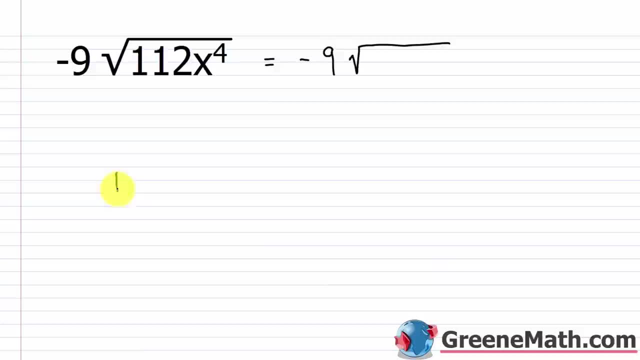 Let's try to break this down inside. And let's just start with the number part. So 112, I know is divisible by two. It's also divisible by four, right? The last two digits would be a 12. So obviously that's divisible by four. It would be four times 28. So let's start with that, 28 times four. Four is a perfect square, it's two times two. 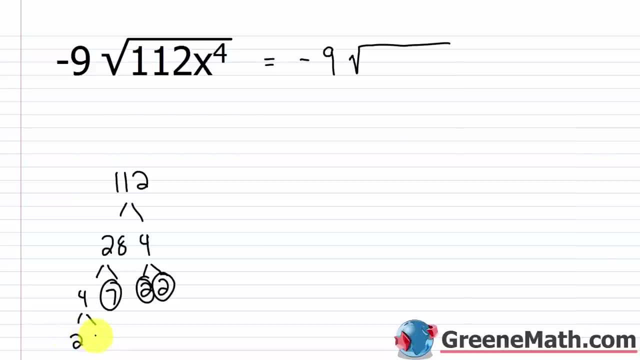 28 is four times seven. Again, four is a perfect square, it's two times two. 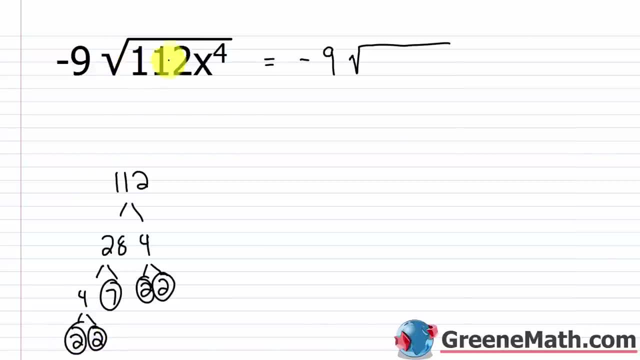 So at this point, I know the number part, the square root of 112 would simplify to what? Two times two, or four, times the square root of seven. 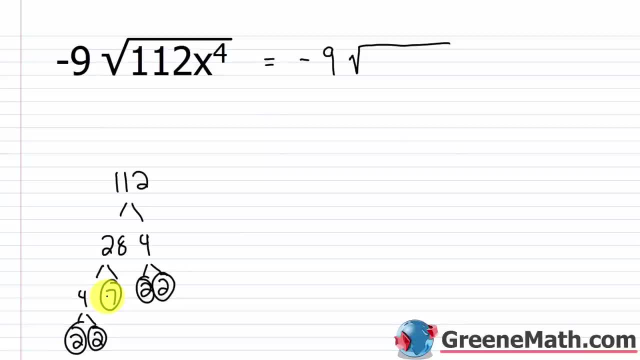 So once you start getting good at this, you can kind of eyeball that and say, okay, I would have four outside of the symbol, and then that would be multiplied by negative nine, and then inside the symbol, for the number part, I'd have a seven. 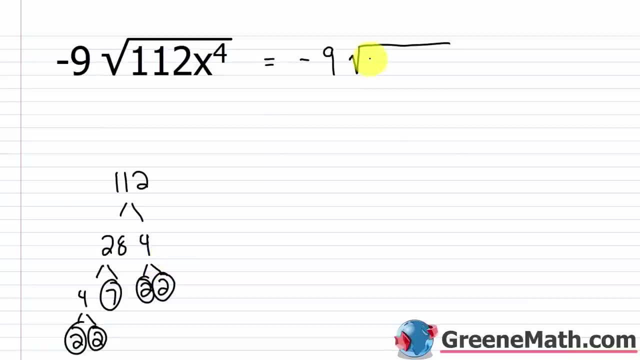 But again, let's kind of slow this down a little bit, and let's write the square root of, four times four is 16, so let's write 16 times seven, and then we have this x to the fourth power to deal with, which we'll think about in a minute. 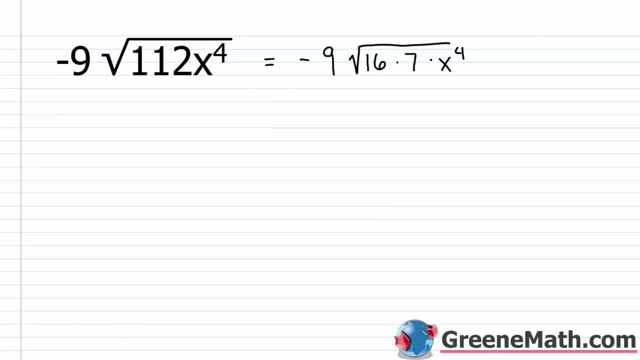 Now, if I look at x to the fourth power, x to the fourth power, this is what? 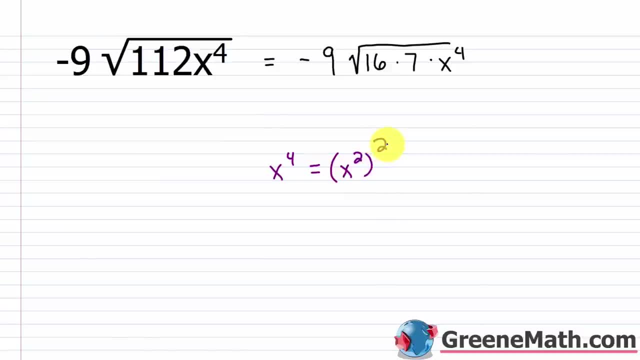 This is x squared, squared. 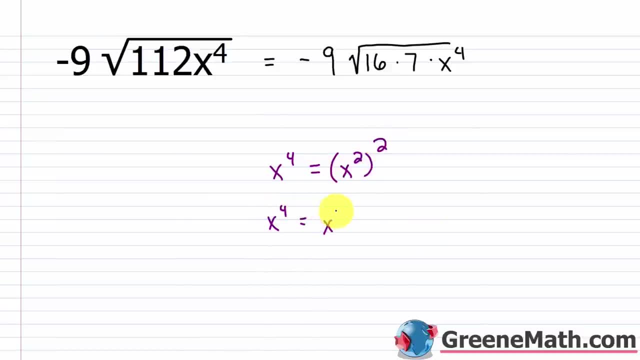 Or I can think about it as, x squared times x squared. X to the fourth power is a perfect square, it's x squared squared. So if I took the square root, if I took the square root of x to the fourth power, this would be equal to x squared, right? Because again, I'm looking for what squared gives me x to the fourth power, and the answer to that is x squared. 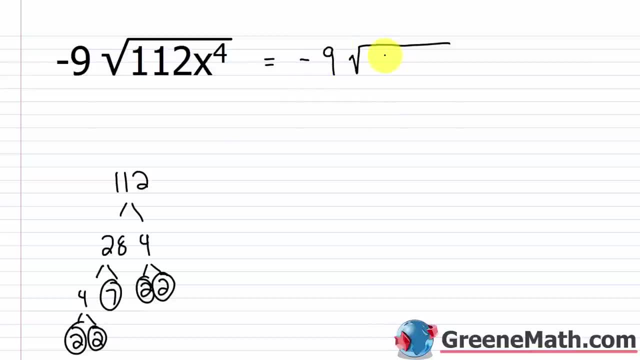 then that would be multiplied by negative 9.. And then inside the symbol for the number part, I'd have a 7.. But again, let's kind of slow this down a little bit and let's write: the square root of 4 times 4 is 16.. So let's write 16 times 7.. And then we have this x to the fourth power. 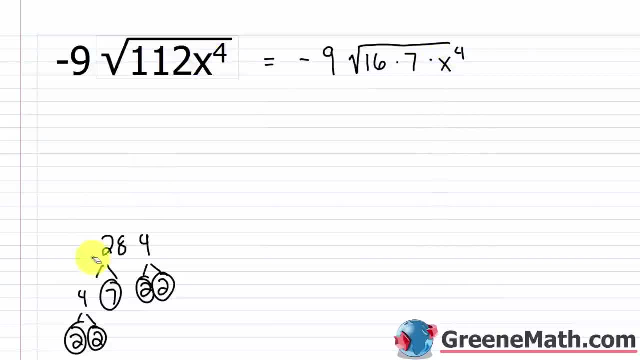 to deal with, which we'll think about in a minute. Now, if I look at x to the fourth power, x to the fourth power, this is what This is: x squared squared. Or I can think about it as x squared times. x squared x to the fourth power is a 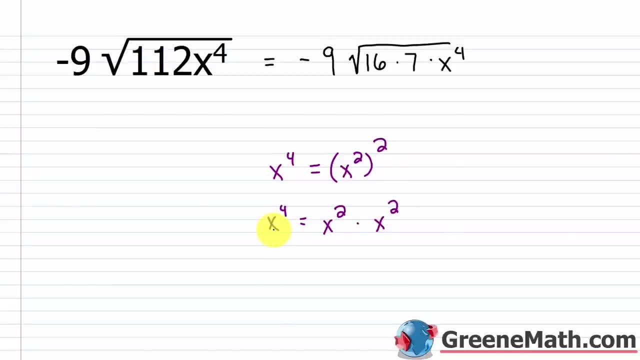 perfect square, It's x squared squared. So if I took the square root, if I took the square root of x to the fourth power, this would be equal to x squared square, right. because again, I'm looking for what squared gives me: x to the fourth power and the 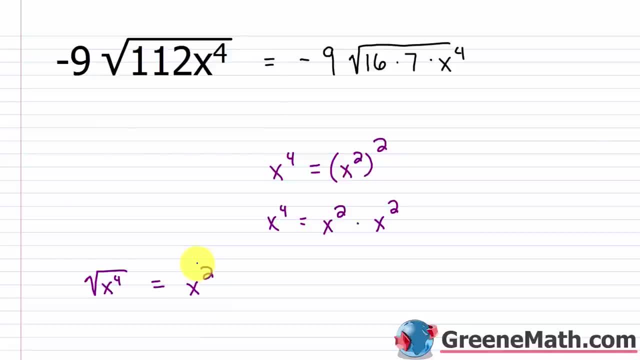 answer to that is x squared, and I know it's a little bit more challenging to understand this when you start dealing with variables and especially with the exponents getting larger and larger. but really it's, it's not too difficult if you just kind of break it down, you know. 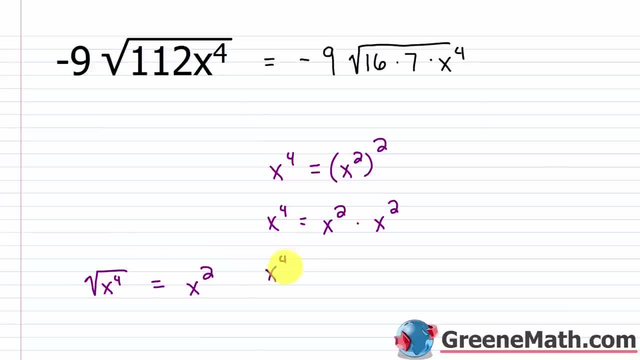 completely into pairs. if I was to say, okay, I have x to the fourth power, and this is x times x times x times x. again, I have one pair of x's, then a second pair of x's, so two of those would kind of come outside the symbol, right, if we did it that way. so this would end up being what x times x or. 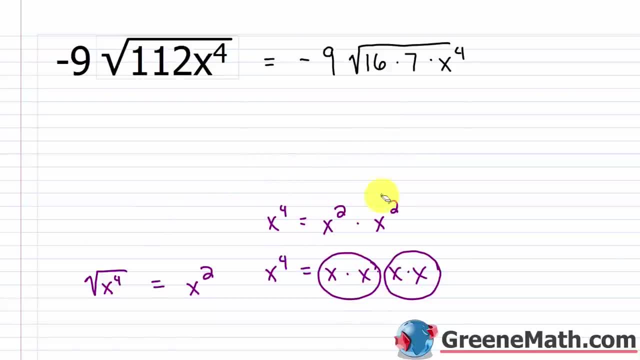 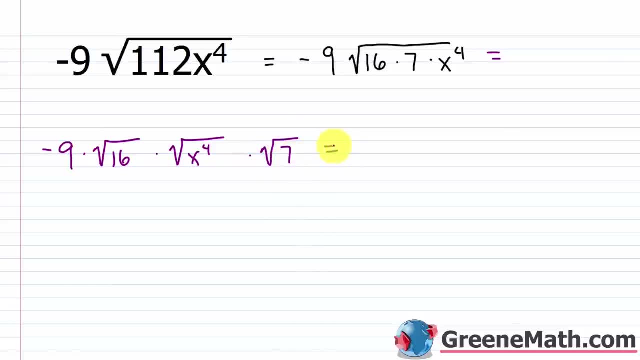 x to the fourth power times the square root of seven. We know that we'd have negative nine times. the square root of 16 is four. the square root of x to the fourth power is x squared, and then the square root of seven. 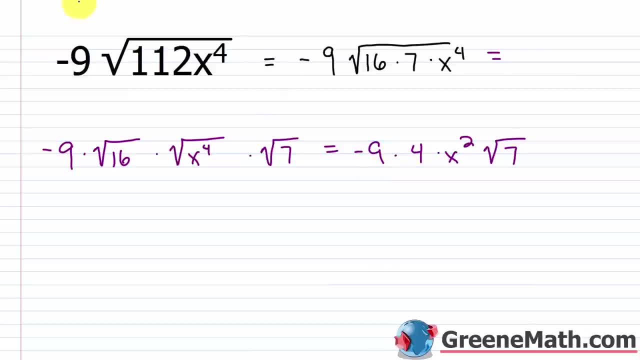 we're not gonna be able to do anything with. So now we just multiply negative nine times four. That's gonna give me negative 36.. Then we have x squared, and then we have times the square root of seven. And if you don't completely understand this example, 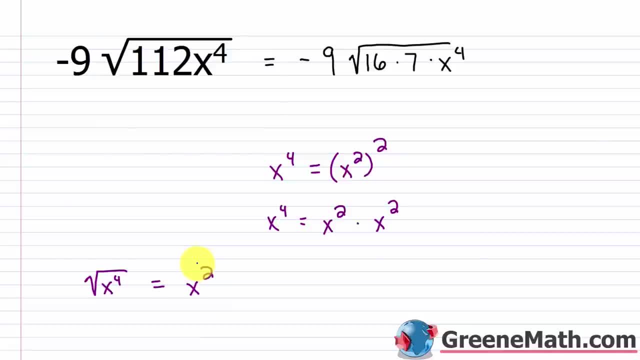 And I know it's a little bit more challenging to understand this when you start dealing with variables, and especially with the exponents getting larger and larger, but really it's not too difficult if you just kind of break it down, you know, completely into pairs. If I was to say, okay, I have x to the fourth power, x times x times x times x, again, I have one pair of x's, then a second pair of x's, so two of those would kind of come outside the symbol, right, if we did it that way. So this would end up being what? X times x or x squared. So let me erase all of this, and I'm gonna just completely break this down now. 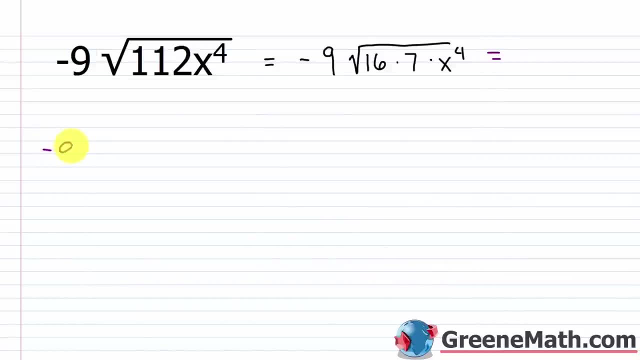 So this is equal to, we have negative nine times the square root of, let's put 16, times the square root of, let's put x to the fourth power, times the square root of seven. 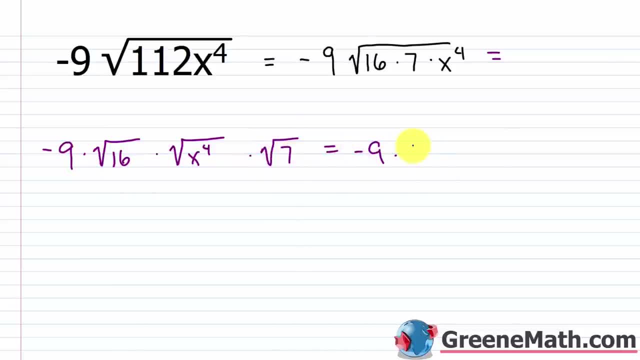 We know that we'd have negative nine times the square root of 16 is four, the square root of x to the fourth power is x squared, and then the square root of seven, we're not gonna be able to do anything with. 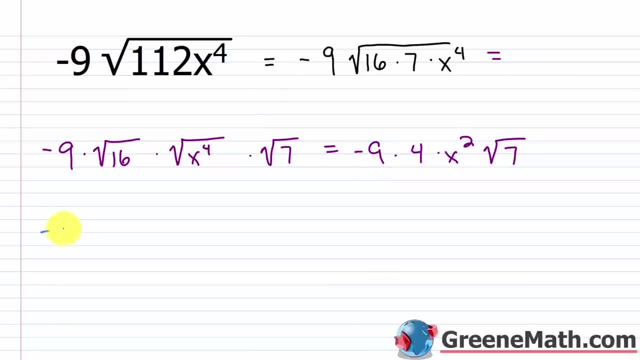 So now we just multiply negative nine times four, and that's gonna give me negative 36. Then we have x squared, and then we have times the square root of seven. 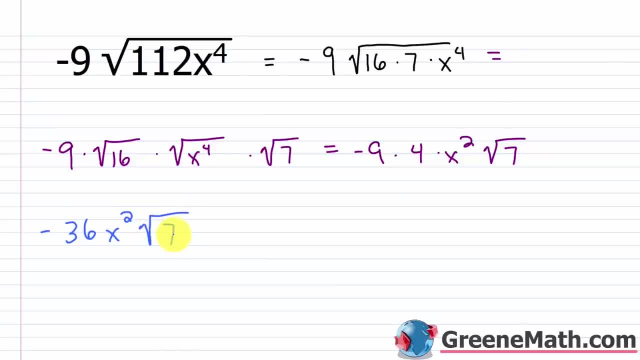 And if you don't completely understand this example, don't feel too bad. 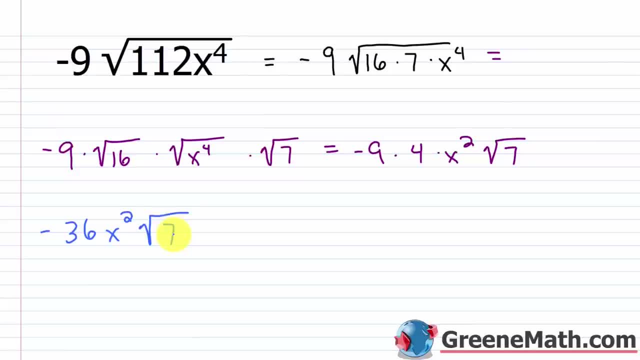 It's one of the more complex ones. You can pause the video, go back, restart the problem, and you can do it in a different way if it's more comfortable for you. 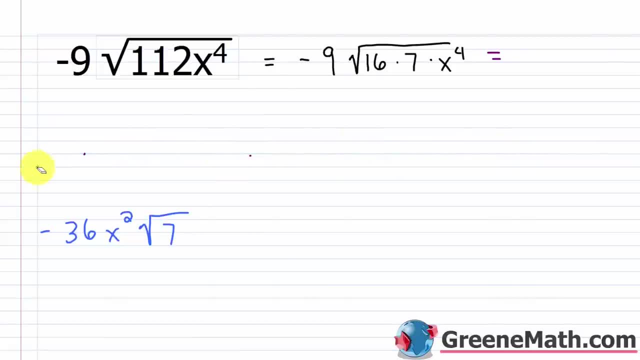 You can, again, let me erase all this. You can completely break this thing down and say, okay, this is negative nine times the square root of four times four times seven times, let's say you did x squared times x squared, or you can even further break this down. 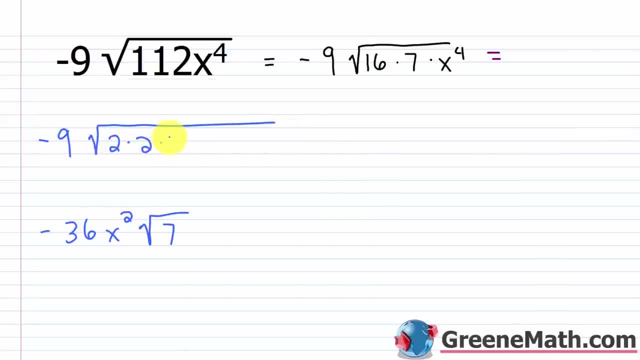 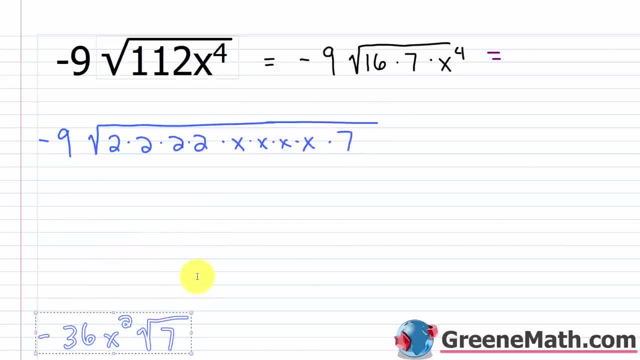 Any way you do this, you're gonna get the same answer. So if this is what makes you feel more comfortable, this is what helps you to understand it, then spend the extra time to do it. 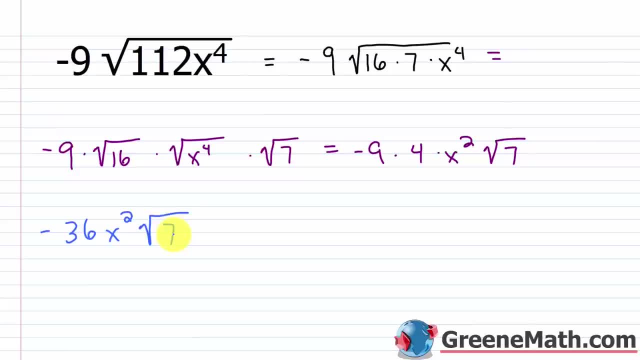 don't feel too bad. It's one of the more complex ones. You can pause the video, go back, restart the problem and you can do it in a different way if it's more comfortable for you. You can again. let me erase all this. 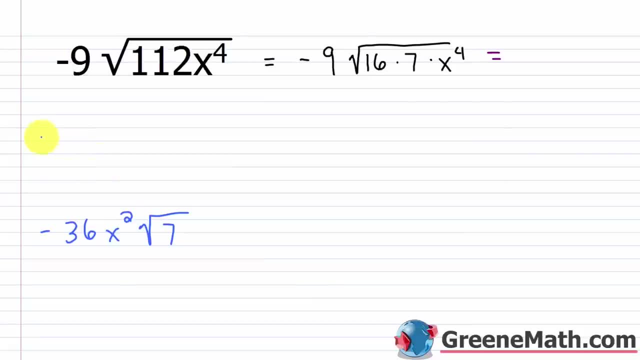 You can completely break this thing down and say, okay, this is negative nine times the square root of four times, four times seven times. let's say you did x squared times x squared. or you can even further break this down all the way and say I have two times two times, two times two. 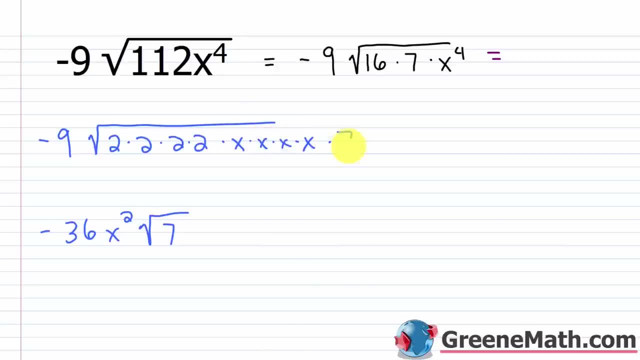 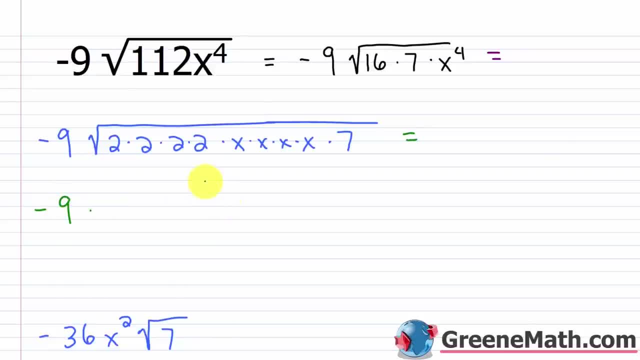 So this is equal to you have negative nine times. remember, for each pair, one's gonna come out. So this would be a two coming out. This would be another two coming out. This would be an x coming out. This would be another x coming out. 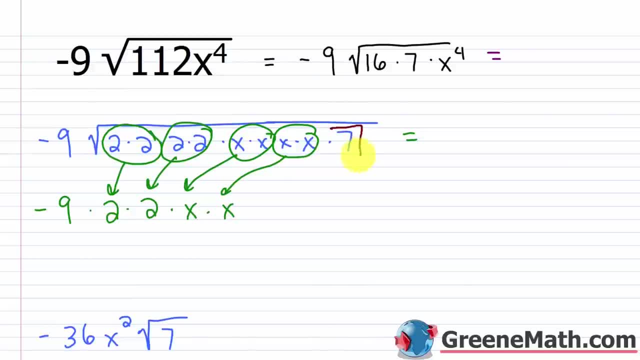 And then the seven would stay in there. So let me put a box around that, And so this would be times the square root of seven. So this equals one. Now it's just straight multiplication. Negative nine times two is negative 18.. 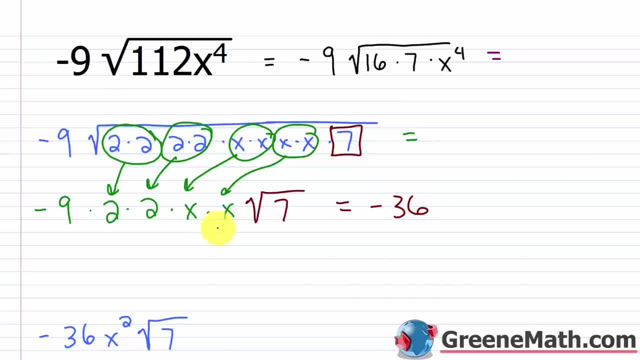 Negative 18 times two is negative 36.. And then for the variables: x times x is x squared, and then times the square root of seven. So our answers match up right. The exact same as this, And this was a little easier to understand, right. 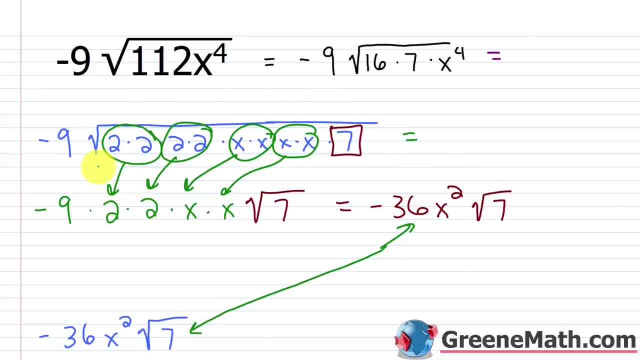 When you first start out again, if you need to spend the extra time to break it down completely, go ahead and do it And then, as you get better, as you get a better understanding, you're going to be able to speed up the process. 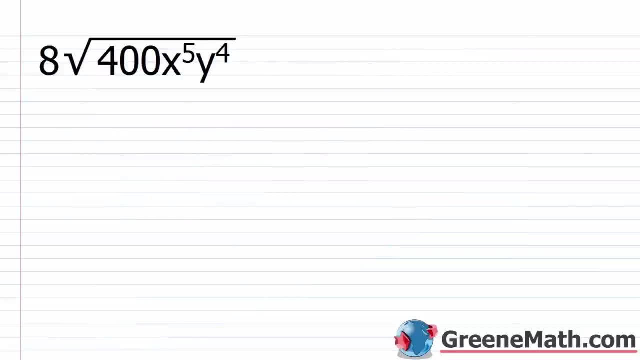 and go very quickly on these problems. All right, let's look at another kind of hard example. So we have eight times the square root of 400: x to the fifth power, y to the fourth power. So we have eight times the square root of six. 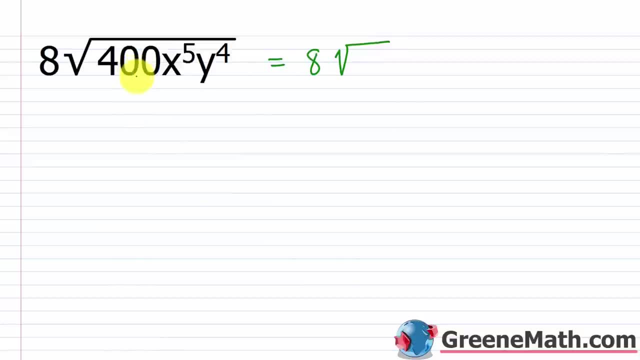 So we have eight times the square root of six root. I know the square root of 400 is 20, so let's just write the square root of 400 times the square root of x to the fifth power times the square root of y to the fourth power. now again, I just 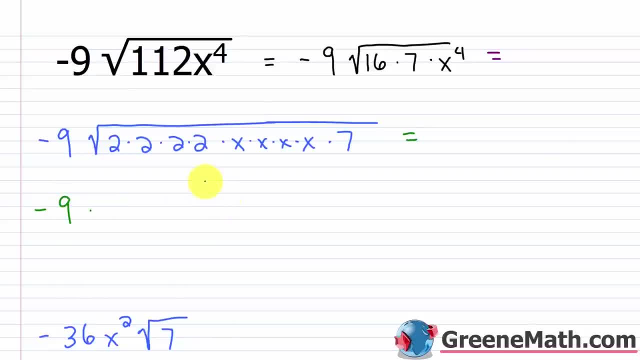 So this is equal to, you have negative nine times, remember for each pair, one's gonna come out. So this would be a two coming out. 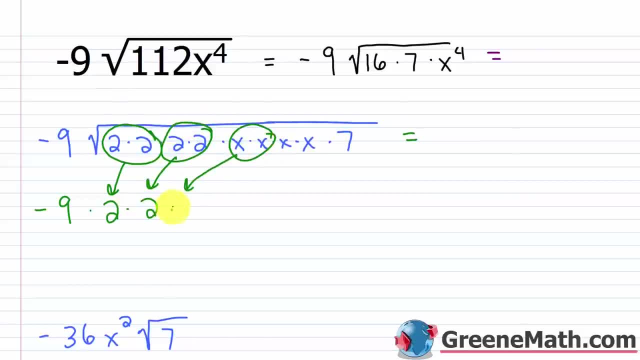 This would be another two coming out. This would be an x coming out. This would be another x coming out. And then the seven would stay in there. 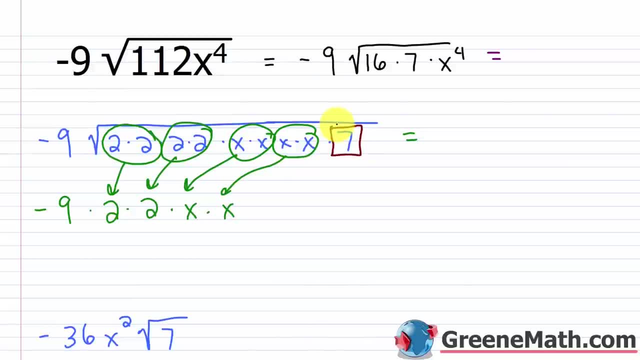 So let me put a box around that. And so this would be times the square root of seven. So this equals one. Now it's just straight multiplication. Negative nine times two is negative 18. Negative 18 times two is negative 36. 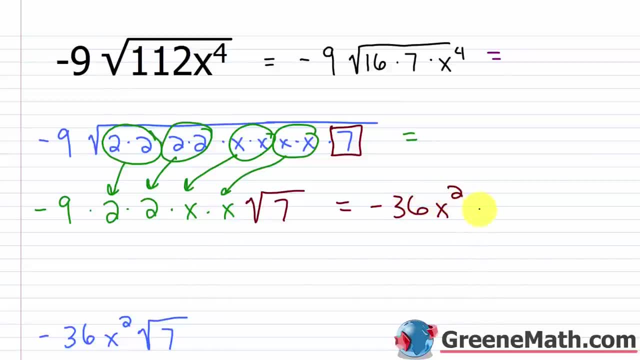 And then for the variables, x times x is x squared, and then times the square root of seven. So our answers match up, right? 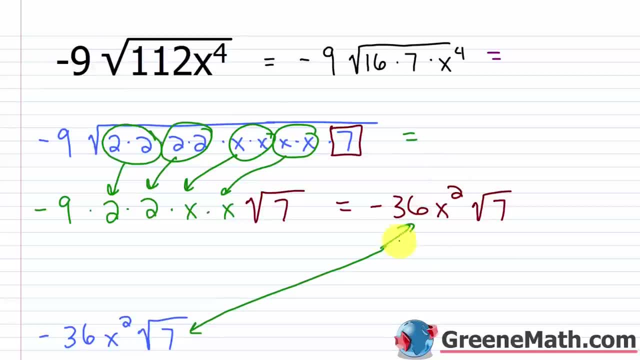 This is the exact same as this. And this was a little easier to understand, right? When you first start out, again, 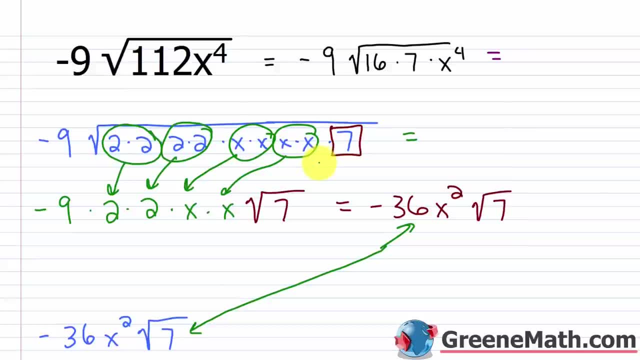 if you need to spend the extra time to break it down completely, go ahead and do it. 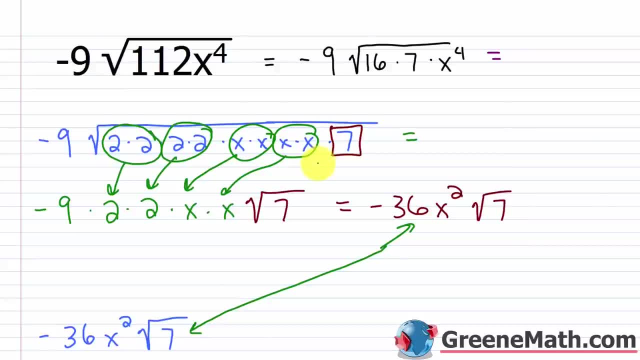 And then as you get better, as you get a better understanding, you're going to be able to speed up the process and go very quickly on these problems. 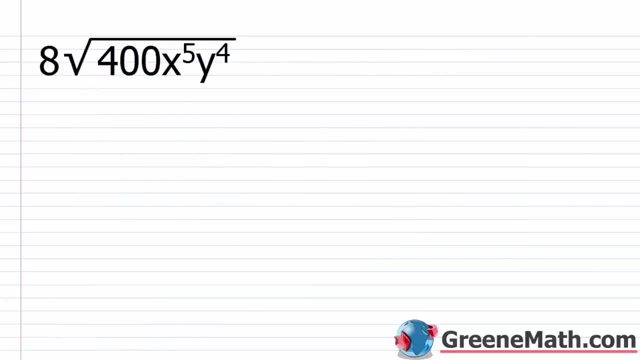 All right, let's look at another kind of hard example. So we have eight times the square root of 400x to the fifth power, y to the fourth power. So we have eight times the square root. I know the square root of 400 is 20. 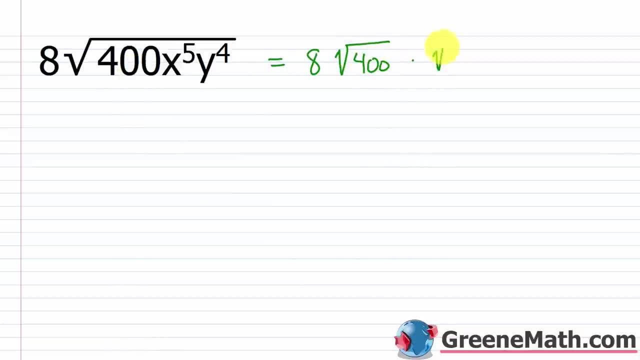 So let's just write the square root of 400 times the square root of x to the fifth power times the square root of y to the fourth power. 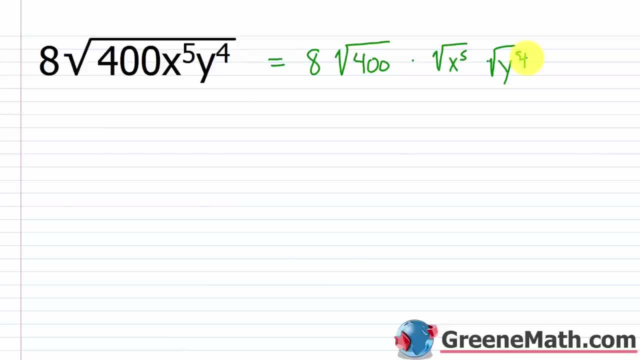 Now, again, I just said the square root of 400 is 20. So let's write equals eight times 20. So we've got that part figured out. 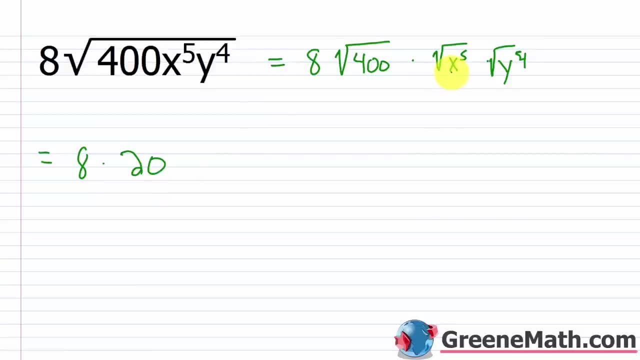 What about x to the fifth power? Well, again, there's multiple ways to kind of think about this. 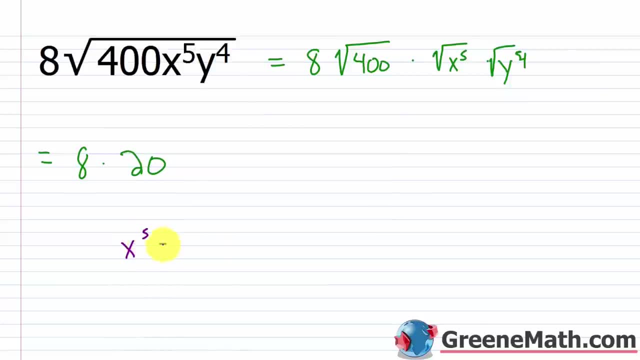 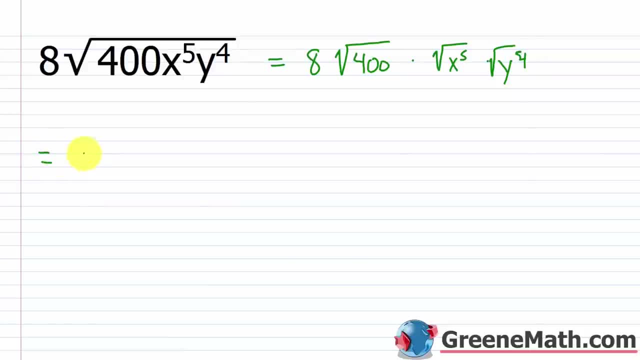 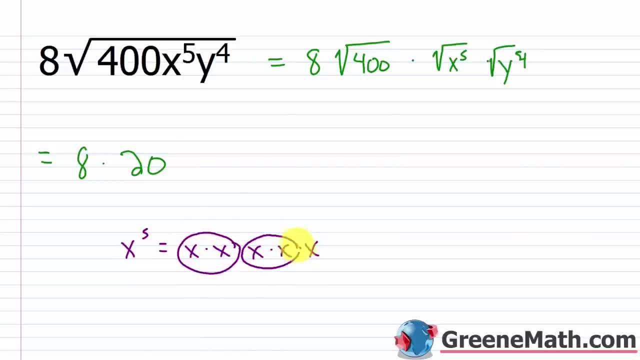 and then for each pair I'm pulling one out. so that means I'd pull out two of these guys. that would be x squared. that's the first kind of way you can think about it. the second way is just thinking about exponents in general. so I know that if I have a square root I'm looking for kind. 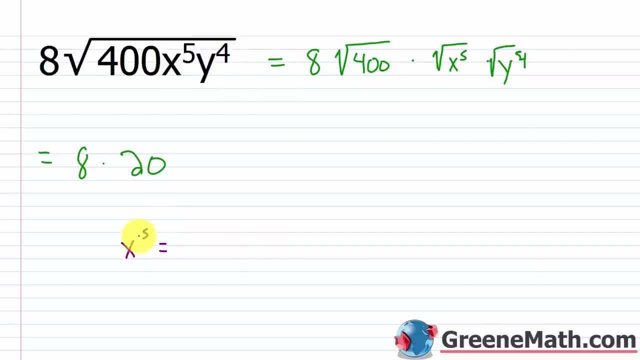 of an even value here, right, it's got to be something that's going to be divisible by two. so if I have a square root, I'm looking for an even value here. right, it's got to be something that's. If I wrote this as x to the fourth power times x to the first power, I know that I could. 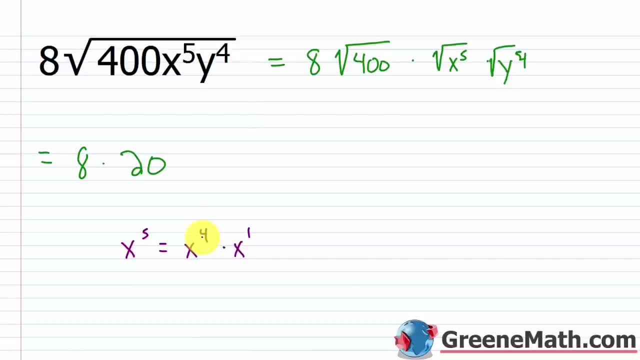 take four and divide it by two, right? So I know I could get two x squareds out of this guy, right? So this could be x squared squared times, x to the first power. And again, when you think about it this way, and it's very, very simple at this point, 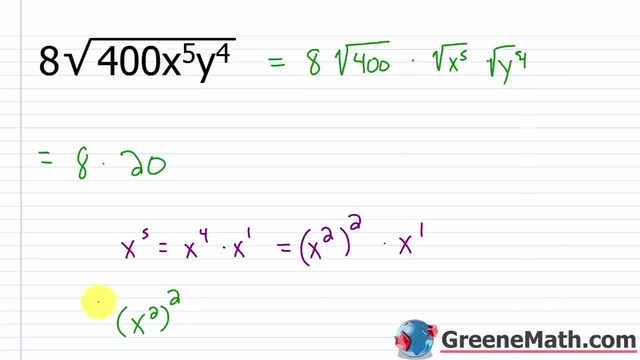 if I have x squared and that's squared, and then I take the square root of this whole thing again. this is going to cancel with this and I'm left with this. just the x squared, So kind of. either way you want to look at that, you would have x squared here and then 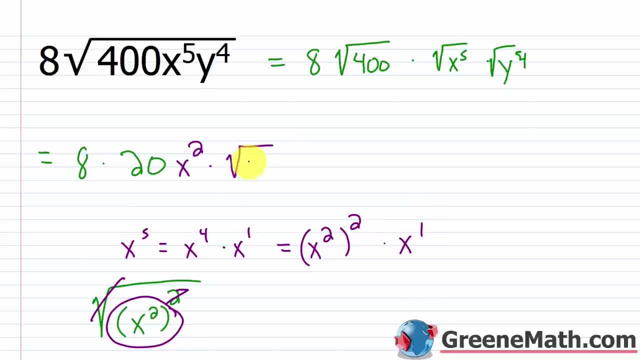 times the square root of, you'd have x to the first power. Now I still have y to the fourth power to deal with, but again, when we start thinking about exponents, very, very quickly, you're going to memorize. 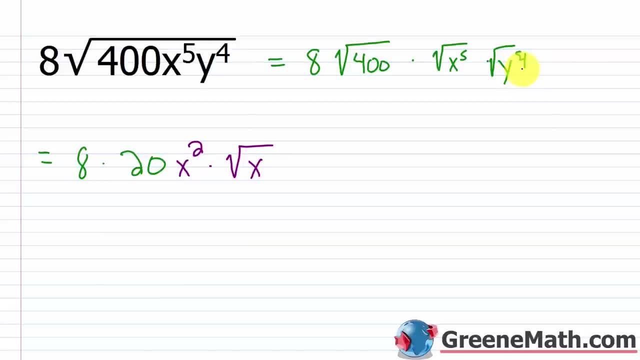 Okay, The square root of something raised to the fourth power is that variable squared. So the square root of y to the fourth power is y squared, right. So let me kind of scooch this down a little bit and put that this is times y squared. 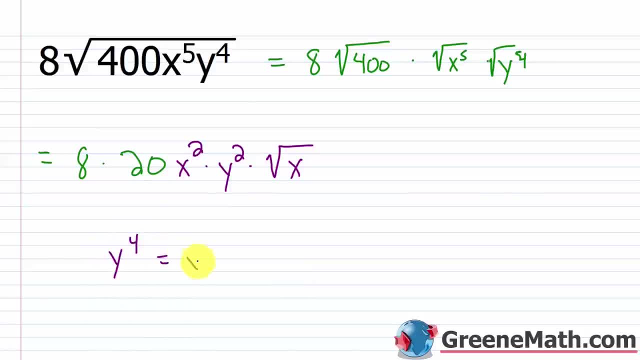 And again, why is that the case? Well, if I have y to the fourth, power is equal to y times y times y times y. for each pair one's going to come out, So two of these come out. So y times y is y squared. 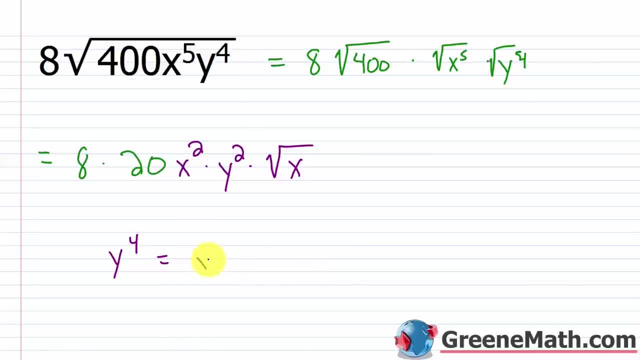 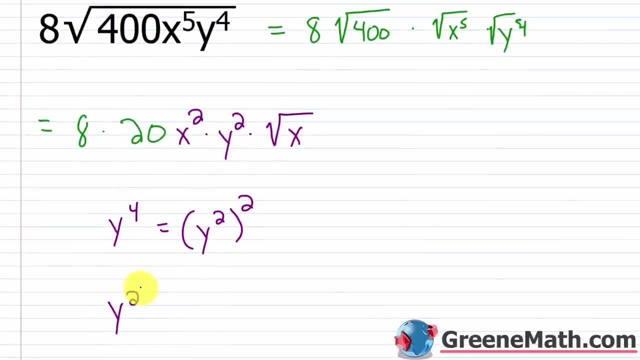 Again, if you wanted to, you could write this as y squared, Y squared, squared, and just think about this being under the square root symbol. Well, of course, if I had y squared, and that was squared, if I took the square root of 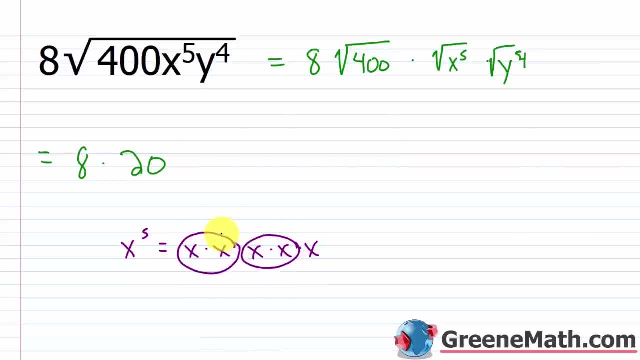 And then for each pair, I'm pulling one out. So that means I'd pull out two of these guys. That would be x squared. That's the first kind of way you can think about it. 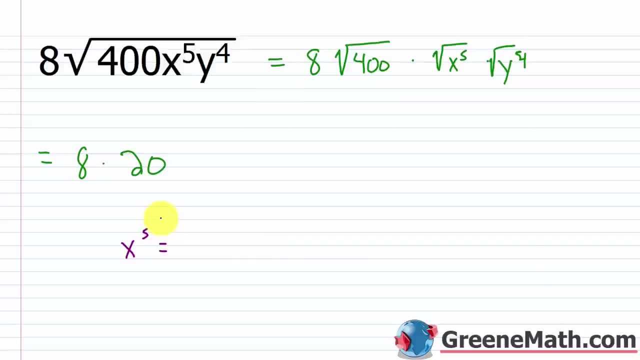 The second way is just thinking about exponents in general. So I know that if I have a square root, I'm looking for kind of an even value here, right? It's got to be something that's going to be divisible by two. 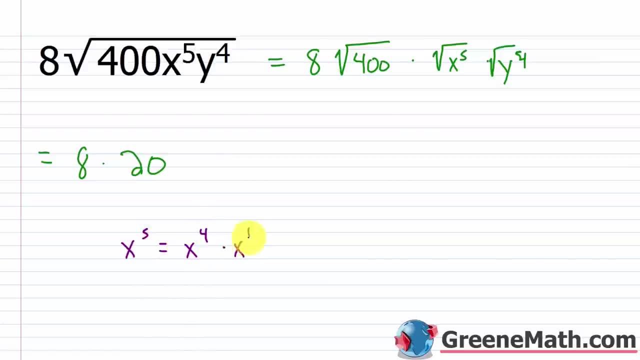 So if I wrote this as x to the fourth power times x to the first power, I know that I could take four and divide it by two, right? So I know I could get two x squareds out of this guy. Right? 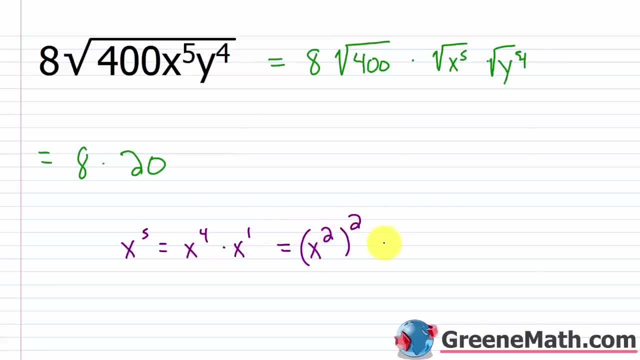 So this can be x squared, squared times x to the first power. And again, when you think about it this way, and it's very, very simple at this point, if I have x squared and that's squared, and then I take the square root of this whole thing, thing, again, this is going to cancel with this and I'm left with this, just the x squared. So 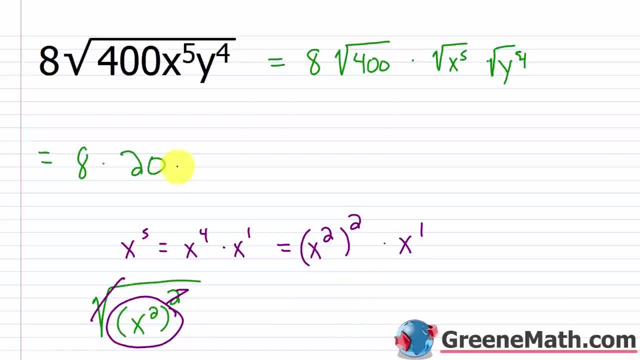 kind of either way you want to look at that, you would have x squared here and then times the square root of, you'd have x to the first power. Now, I still have y to the fourth power to deal with. But again, when we start thinking about exponents, very, very quickly, you're going to 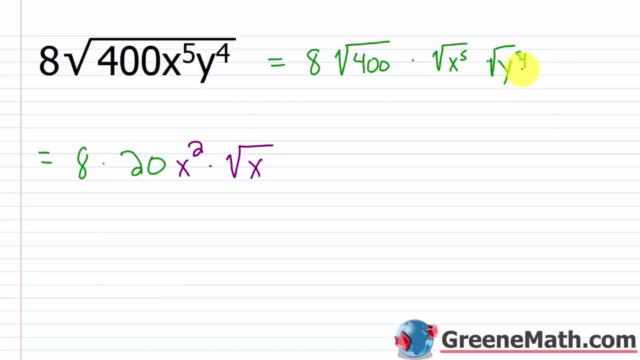 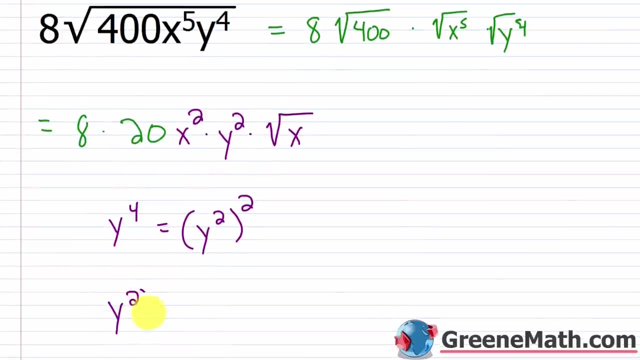 memorize the square root of something raised to the fourth power is that variable squared. So the square root of y to the fourth power is y squared. So let me kind of scooch this down a little bit and put that this is times y squared. And again, why is that the case? Well, if I have y to the fourth power is equal to y times y times y times y, for each pair, one's going to come out. So two of these come out. So y times y is y squared. Again, if you wanted to, you could write this as y squared squared. And just think about this being under the square root symbol. Well, of course, if I had y squared, and that was squared, if I took the square root of this guy, this would cancel with this, and I'd be left with y squared. So you do whatever you have to do to understand this at first. Again, when we get to kind of fractional exponents, we're going to have some methods that are going to really speed our work up here. 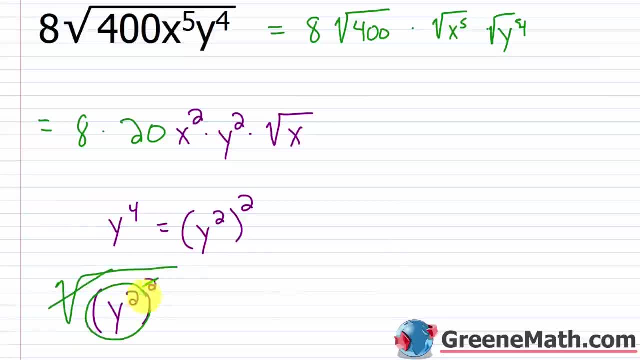 this guy. this would cancel with this and I'd be left with y squared. So you do whatever you have to do to understand this at first. Again, when we get to kind of fractional exponents, we're going to have some methods that are: 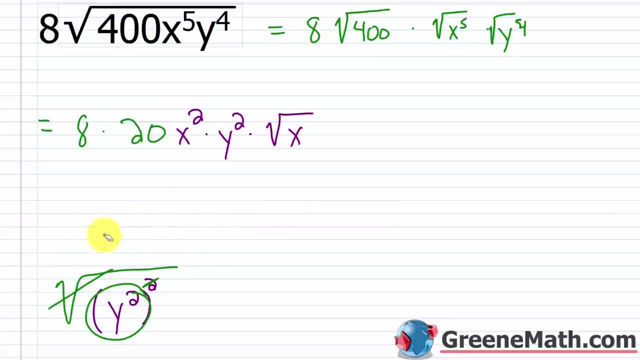 going to really speed our work up here, But for right now, again, we do what we have to do. And so 8 times 20 is our y, 8 times 20 is 160.. And then times x squared, times y squared, and then times the square root of x. 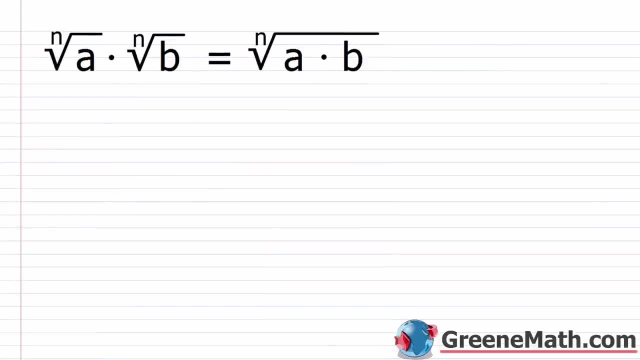 Alright. so the last thing I want to do, and this might not come up in Algebra 1.. You might have to wait till you get to Algebra 2 to kind of see these problems, But it might come up in your course, so I want to cover it. 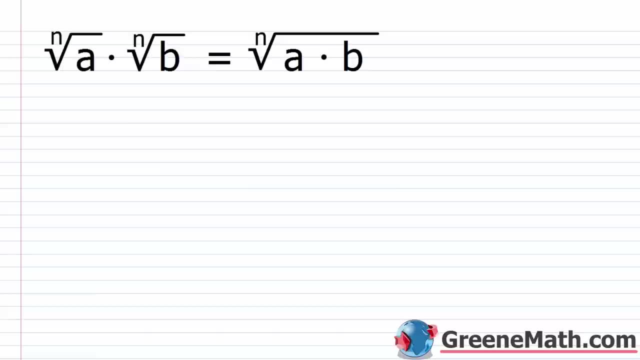 You have higher roots that you can apply these techniques to. So if I have the nth root of a times the nth root of b, I'm able to say this is equal to the nth root of a times b. So, in other words, if I have the nth root of a times the nth root of b, I'm able to. 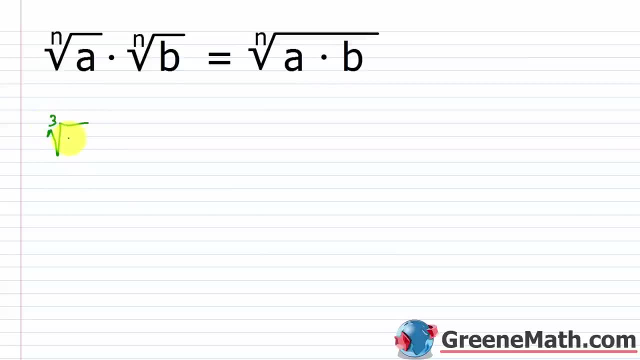 say, this is equal to the cube root of 27 times the cube root of, let's say, 8.. This is equal to the cube root of 27 times 8, which would be the cube root of 216.. Now, again, this is something we can check. 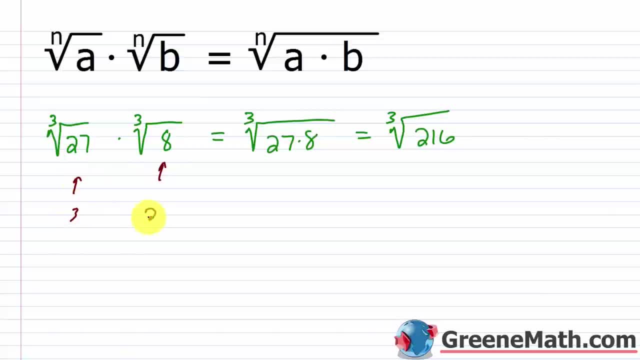 The cube root of 27 is 3.. The cube root of 8 is 2.. So 3 times 2 should give me 6.. The cube root of 216 is 6.. 6 times 6 is 36.. 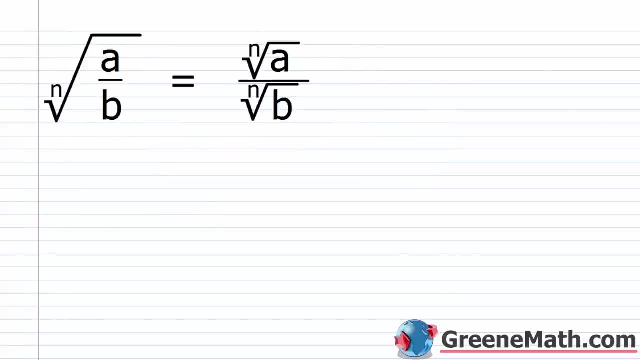 36 times 6 is 216.. Same thing for the quotient rule. The nth root of a over b is equal to the nth root of a over the nth root of b. So, for example, if I had something like: let's say, the fourth root of 1 16th is equal to: 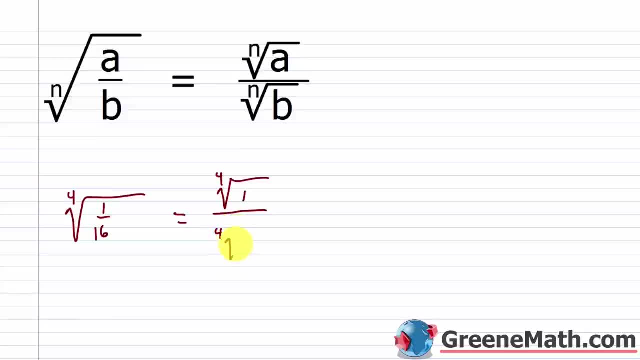 the fourth root of 1 over the fourth root of 16.. And the fourth root of 1 is 1.. The fourth root of 16 is 2.. So this would be 1 half And of course you can prove this. 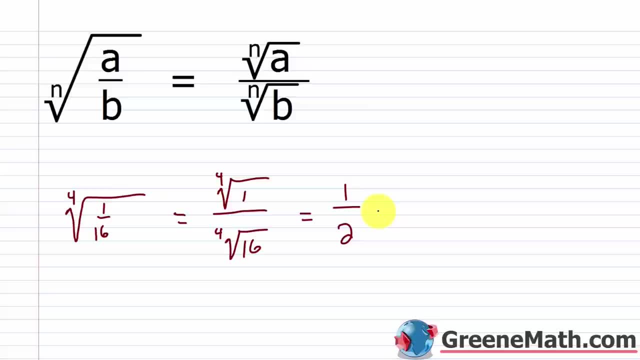 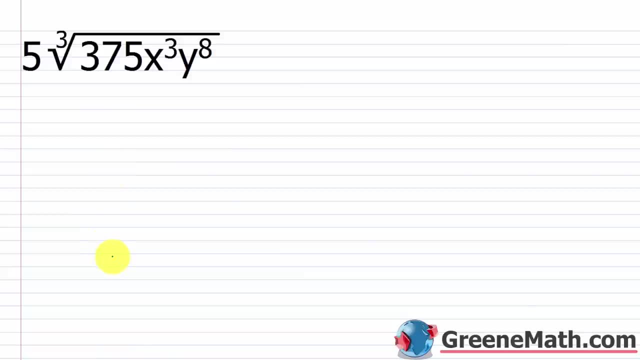 One half times one half Is 1 fourth. 1 fourth times 1 half is 1 eighth, And 1 eighth times 1 half is 1 16th. All right, so let's take a look at a few examples here. 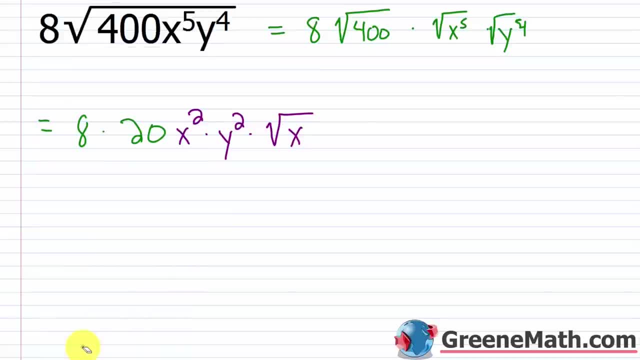 But for right now, again, we do what we have to do. And so 8 times 20 is 160. And then times x squared times y squared. 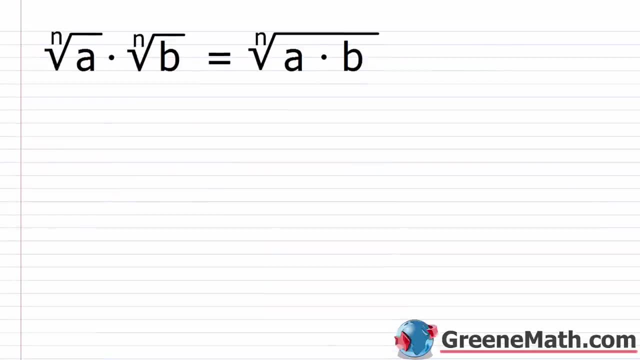 And then times the square root of x. All right, so the last thing I want to do, and this might not come up in Algebra 1, you might have to wait till you get to Algebra 2 to kind of 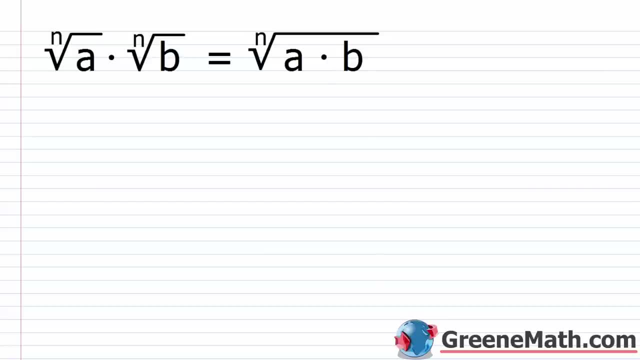 see these problems. But it might come up in your course, so I want to cover it. You have higher 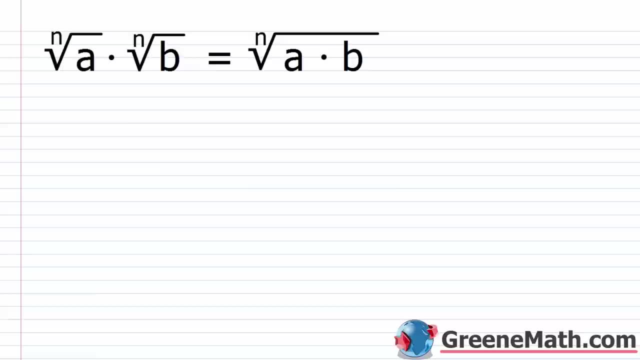 roots that you can apply these techniques to. So if I have the nth root of a times the nth root of b, 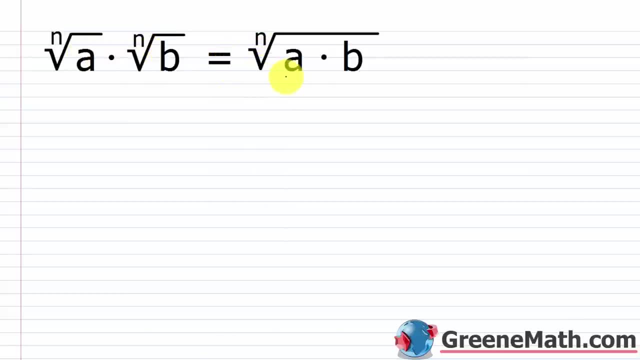 I'm able to say this is equal to the nth root of a times b. So in other words, if I had the cube root of 27 times 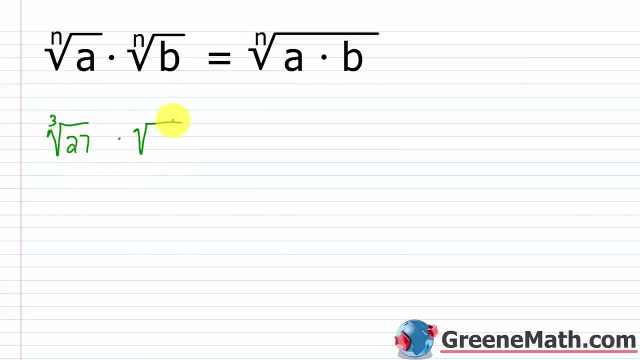 the cube root of, let's say, 8, this is equal to the cube root of 27 times 8, which would be the 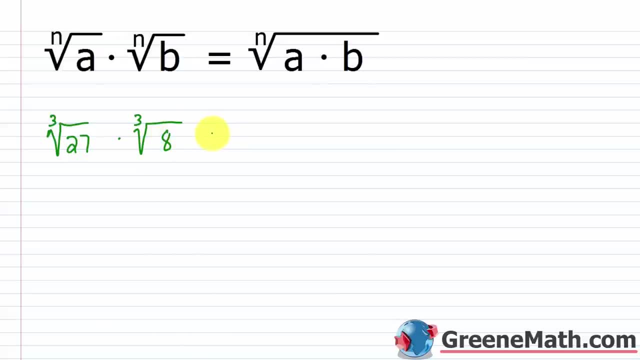 cube root of 260. Now, again, this is something we can check. The cube root of 27 is 3. The cube 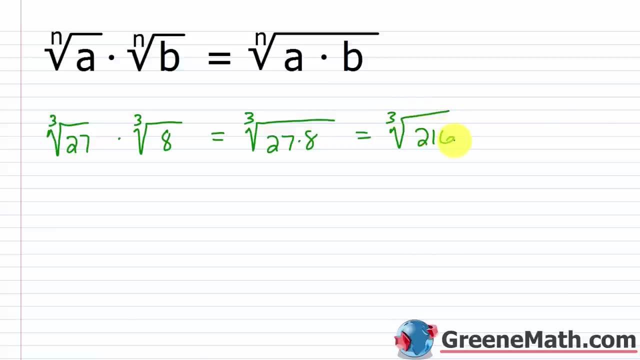 root of 8 is 2. So 3 times 2 should give me 6. The cube root of 216 is 6. 6 times 6 is 36. 36 times 6 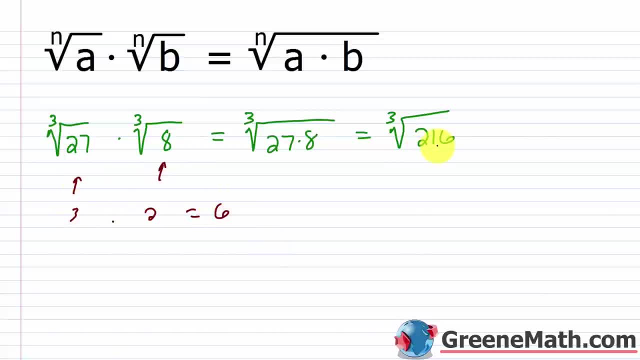 is 216. Same thing for the quotient rule. 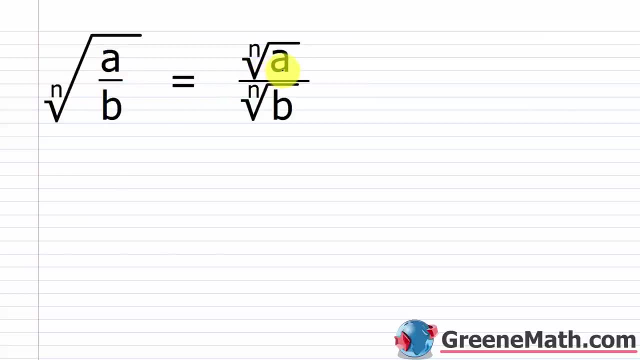 The nth root of a over b is equal to the nth root of a over the nth root of b. So for example, if I had something like, let's say, the fourth root of 116, this is equal to the fourth root of 1 over the fourth root of 16. And the fourth root of 1 is 1. The fourth root of 16 is 2. So this 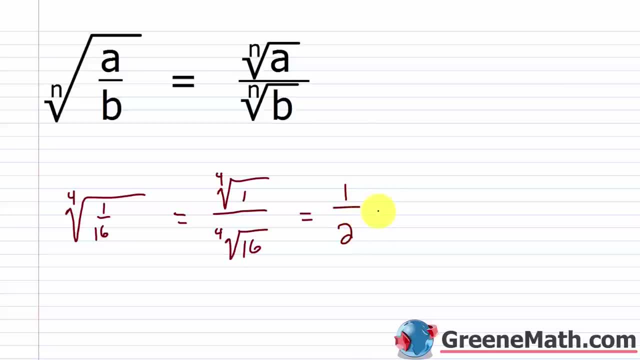 would be 1 half. And of course, you can prove this. 1 half times 1 half is 1 fourth. 1 fourth 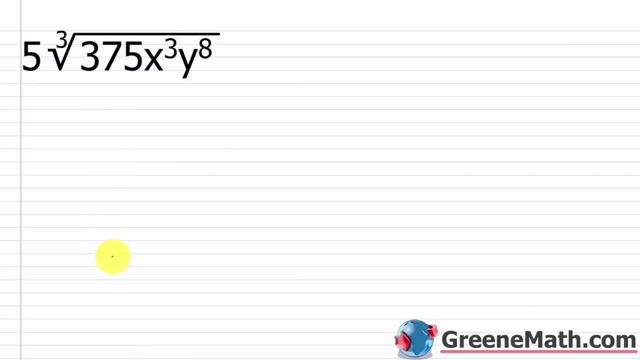 16. All right. So let's take a look at a few examples here. And these are going to be pretty challenging. So don't feel overwhelmed if you can't get them right away. So we have 5 times the cube root of 375 times x cubed times y to the eighth power. So the first thing I'm going to do is break down 375. And I'm going to be looking for perfect cubes now. And when we talked about 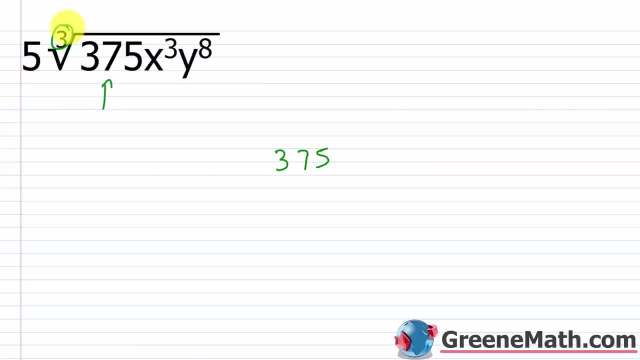 a perfect square, it was a number whose square root was a rational number. 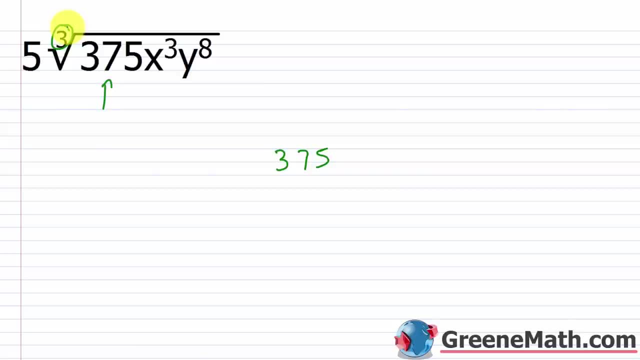 So for a perfect cube, it's a number whose cube root is a rational number. So for example, 8 is a perfect cube, right? Its cube root is 2. That's a rational number. Or 1 eighth is a perfect cube, right? Its cube root is 1 half, which is a rational number. So for 375, I notice it ends in 5. So I can go ahead and divide by 5. And I find this would be 5 times 75. So 5 is prime. Let's circle that. And then 75 is a perfect cube. So I can go ahead and divide by 5. And I find this would 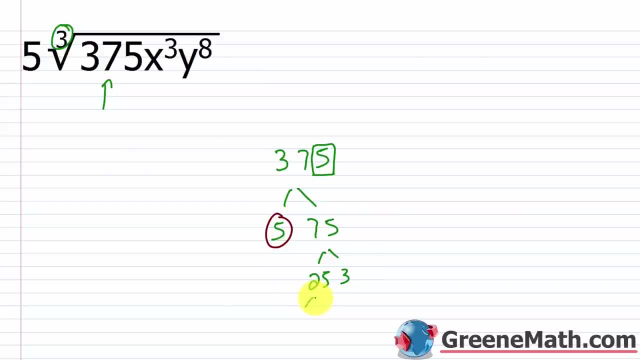 is what? It's 25 times 3. And 25 is 5 times 5. So these are all going to be prime. And I have a perfect cube here. I have 5 times 5 times 5. So 5 cubed or 125 times 3 is how I 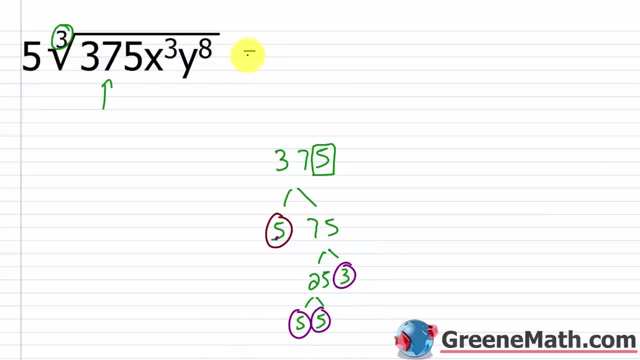 could break down 375. So let's start with that. So let's say this is 5 times the cube root of, and I'm just going to write 125, and then times the cube root of 3, and then times, if I have x cubed and I take the cube root of that, that's just going to be x. If I have an exponent of 3 and I have an index of 3, those are going to cancel each other out. And again, we're going to learn that when we get to fractional exponents. If I have the cube root of something, it's like raising it to the power of one third. So if I had x cubed and it was raised to the power of one third, that's going to be x cubed. So if I have x cubed and it was raised to the power of one third, this would be equal to x, base stays the same, multiply exponents. 3 times 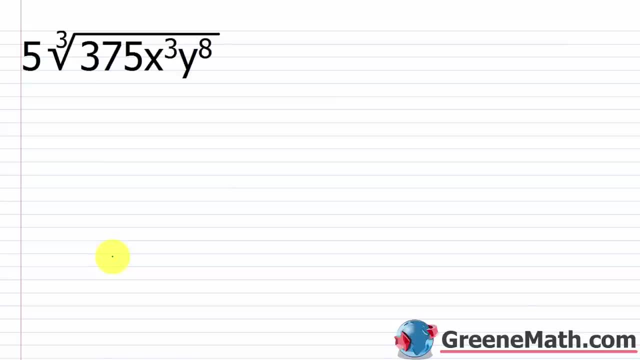 And these are going to be pretty challenging, So don't feel overwhelmed if you can't get them right away. So we have 5 times the cube root of 375, times x, cubed times y to the eighth power. So the first thing I'm going to do is break down 375. 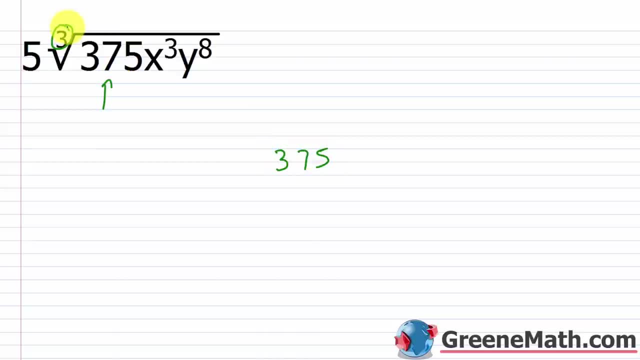 And I'm going to be looking for perfect cubes now. And when we talked about a perfect square, it was a number whose square root was a rational number. So for a perfect cube, it's a number whose cube root is a rational number. 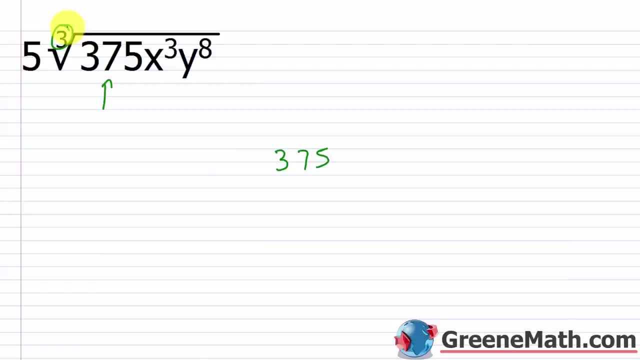 So, for example, 8 is a perfect cube. Its cube root is 2.. That's a rational number. Or 1, eighth is a perfect cube. Its cube root is 1, half, which is a rational number. So for 375, I notice it ends in 5.. 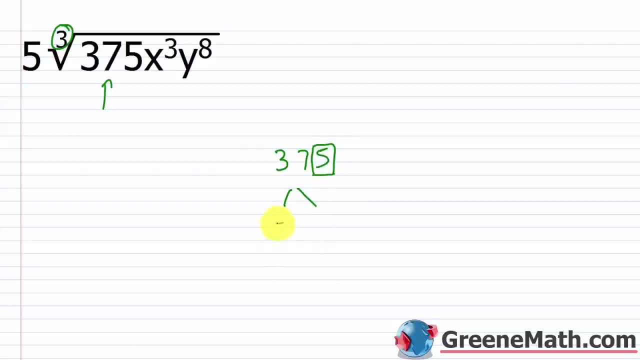 So I can go ahead and divide by 5. And I find this would be 5.5.. So I can go ahead and divide by 5.5.. And this would be 5.5 times 75.. So 5 is prime. 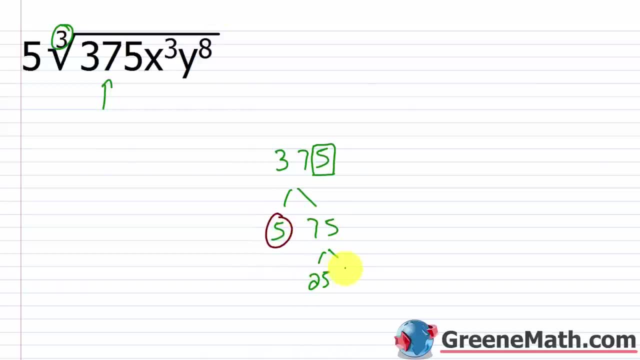 Let's circle that. And then 75 is what It's 25 times 3.. And 25 is 5 times 5.. So these are all going to be prime And I have a perfect cube here. I have 5 times 5 times 5.. 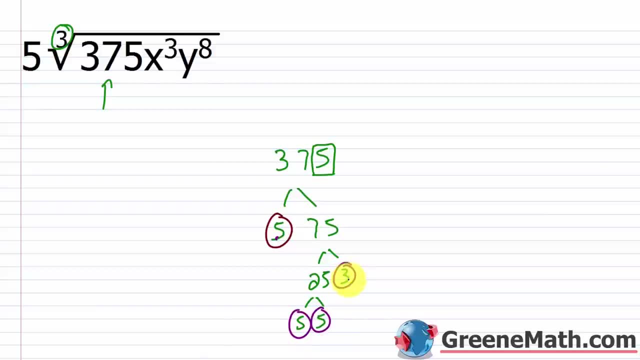 So 5 cubed or 125 times 3 is how I could break down 375.. So let's start with that. So let's say this is 5.5.. times the cube root of- and I'm just going to write 125- and then times the cube root of 3. 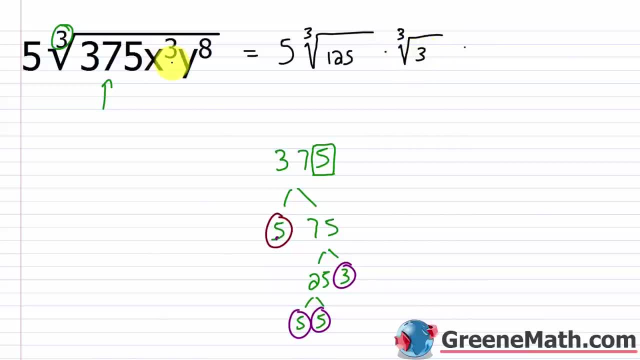 and then times. if I have x cubed and I take the cube root of that, that's just going to be x. If I have an exponent of 3 and I have an index of 3, those are going to cancel each other out and again. 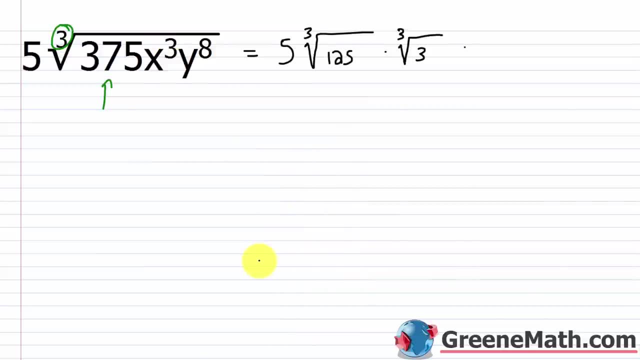 we're going to learn that when we get to fractional exponents, If I have the cube root of something, it's like raising it to the power of 1- 3rd. So if I had x cubed and it was raised to the power of 1, 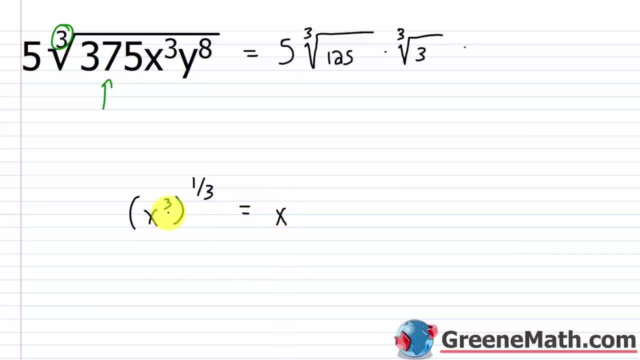 3rd, this would be equal to x. base stays the same. multiply x minus 3 times 1, 3rd is 1.. Okay, but again, we'll learn that in a future lesson, But right now you can just think about it as I have x times x. 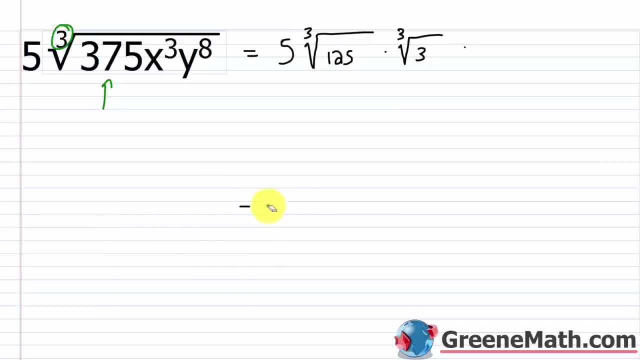 one third is 1. But again, we'll learn that in a future lesson. But right now, you can just think 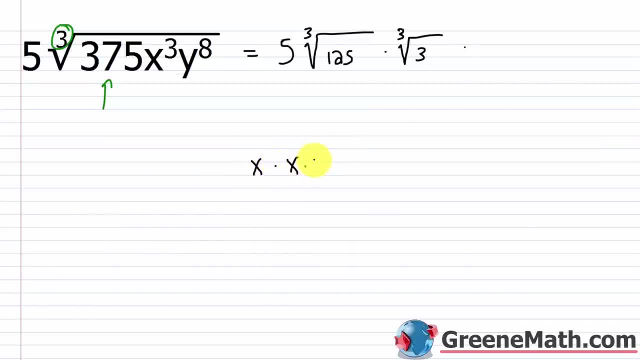 about it as I have x times x times x. That gives me x cubed. So x cubed is a perfect cube. So let's write the cube root of x cubed, and then times. Now I have y to the eighth power. How can we break that down to kind of understand that? So let's start with the cube root of x cubed, and then understand what's going to be able to come out. So now what I'm looking for is a number that's going to be divisible by 3. So the closest one would be 6, right? So if I wrote this as y to the sixth power times y squared, I can think about y to the sixth power as a perfect cube, right? Because if I took the cube root of that, I can think about this as what? y squared times y squared times y squared. That would give me y to the sixth power. So I could write this as the cube root of y squared cubed times the cube root of y squared. And I know I got a lot of stuff going on on the screen. I'm trying to fit it on there. So I'm going to put my equals over here. And then 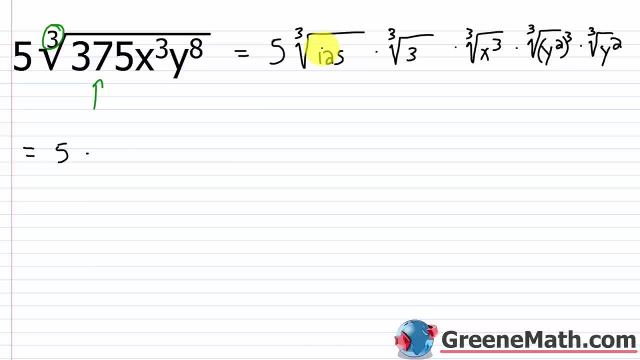 5 times, we know the cube root of 125 is 5. The cube root of 3, I can't really do anything with that. Let me write that way down here. It's just going to stay. Then I have the cube root of x cubed. We know that's x at this point. Then I have the cube root of x cubed. We know that's x at this point. Then I have the cube root of x cubed. We know that's x at this point. Then I have the 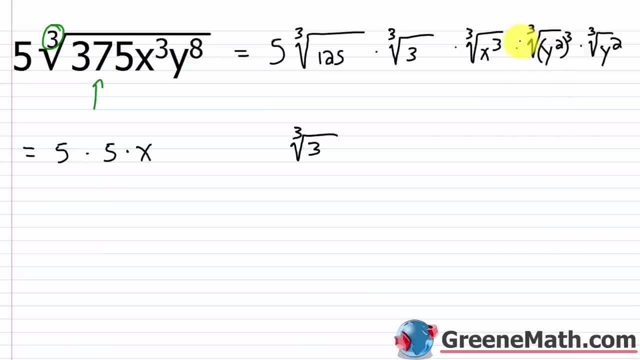 cube root of y squared cubed. So again, this, you can think about this would cancel with this, and I'm left with y squared. So this would just be times y squared. And then I have this times the cube root of y squared. So in the end, what this is going to be equal to, 5 times 5 is 25, 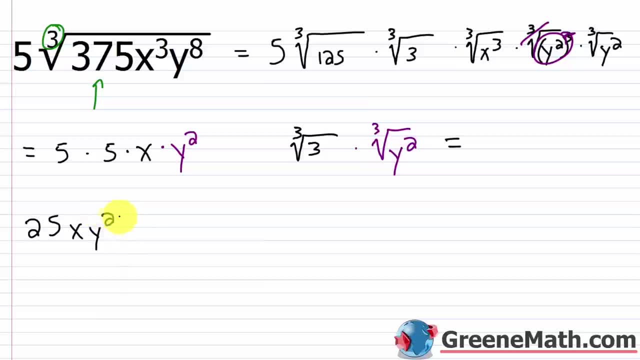 times x times y squared. So xy squared. And then times the cube root of 3y squared. So xy squared. And then times the cube root of 3y squared. And then times the cube root of 3y squared. And all I did was just combine those two that were under the radical symbols. 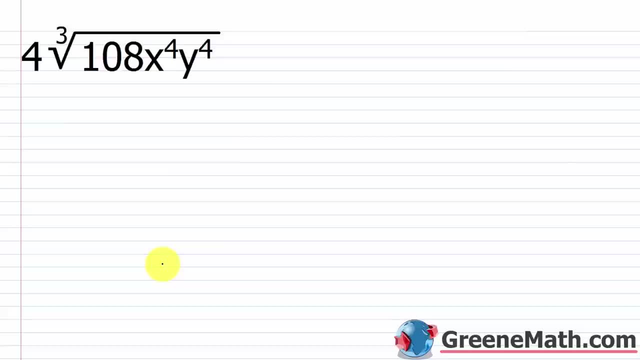 So for the next one, let me look at 4 times the cube root of 108 x to the 4th power y to the 4th power. 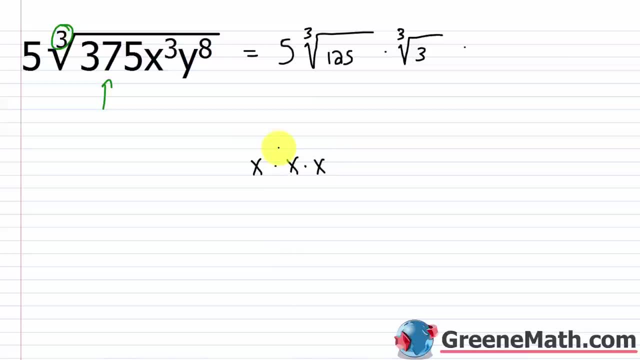 times x, that gives me x cubed. So x cubed is a perfect cube. So let's write the cube root of x cubed and then times. Now I have y to the eighth power. How can we break that down to kind of understand? 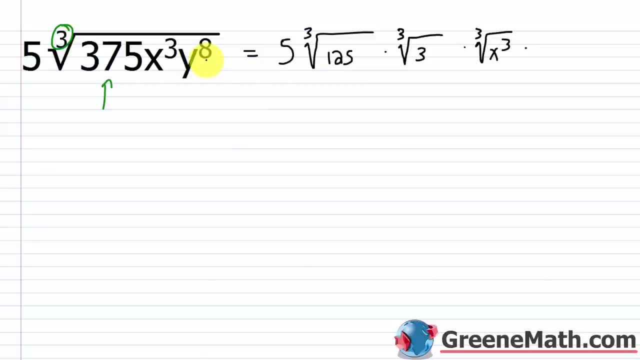 what's going to be able to come out. So now what I'm looking for is a number that's going to be divisible by three, So the closest one would be six, right? So if I wrote this as y to the sixth power, times y squared, I can think about y to the sixth power as a perfect cube, right? Because 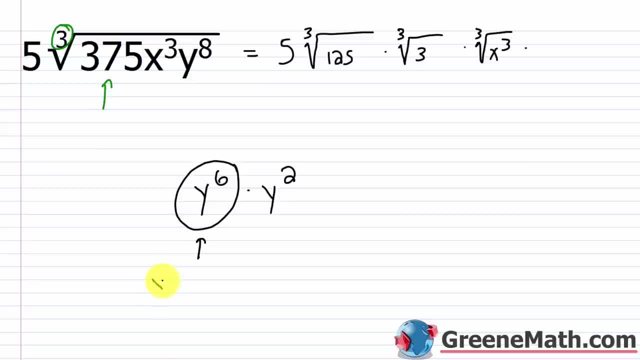 if I took the cube root of that, I can think about this as what: y squared times y squared times y squared, That would give me y to the sixth power. So I could write this as the cube root of y squared, cubed times the cube root of y squared. And I know I got a lot of stuff going. 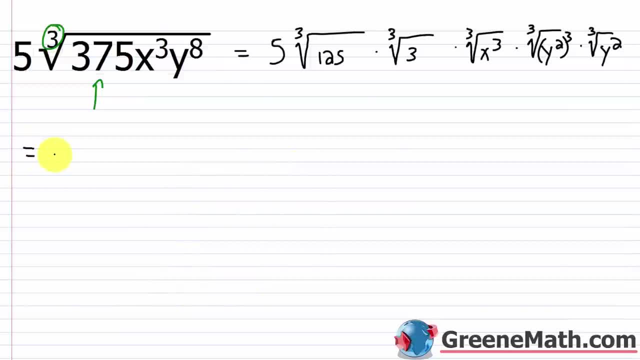 on on the screen. I'm trying to fit it on there, but so I'm going to put my equals over here. and then five times. We know the cube root of 125 is five, The cube root of three. I can't really do. 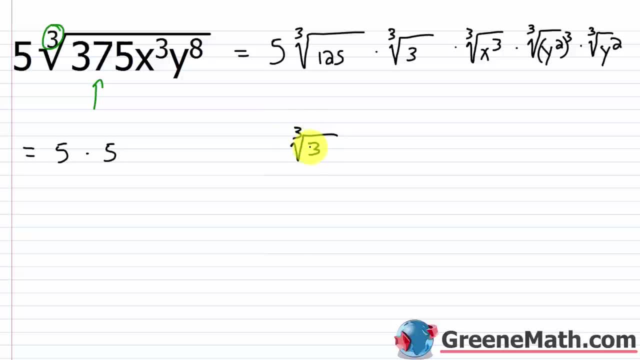 anything with that. Let me write that way down here. I was just going to stay. Then I have the cube root of x cubed. We know that's x at this point. Then I have the cube root of y, squared, cubed. So again, this you can think about, this would. 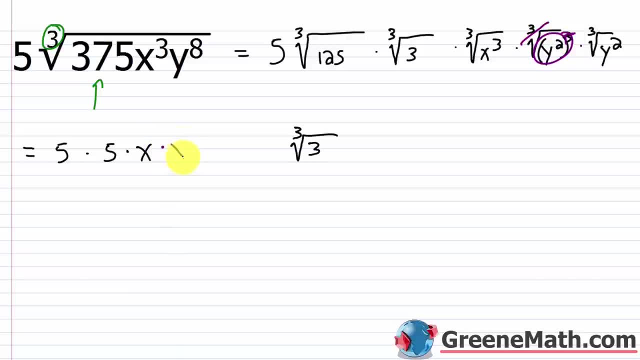 cancel with this and I'm left with y squared. So this would just be times y squared, And then I have this times the cube root of y squared. So in the end, what this is going to be equal to five times five is 25 times x times y squared. So 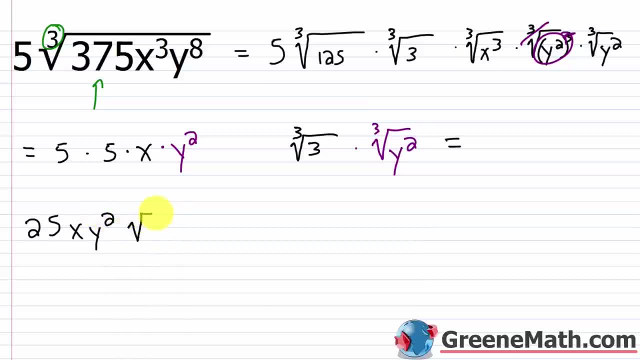 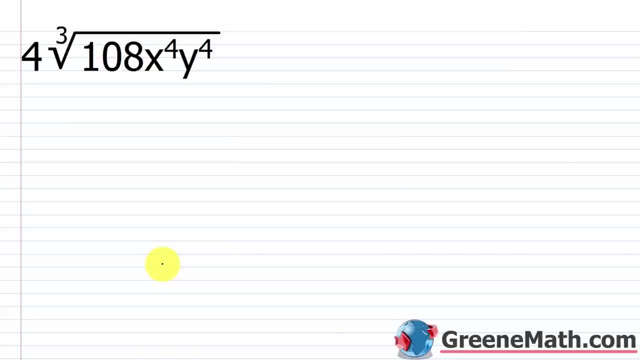 this is going to be x times y squared, And then times the cube root of three y squared, And all I did was just combine those two that were under the radical symbols. So for the next one, let me look at four times the cube root of 108: x to the fourth power, y to the fourth power. So if I broke down, 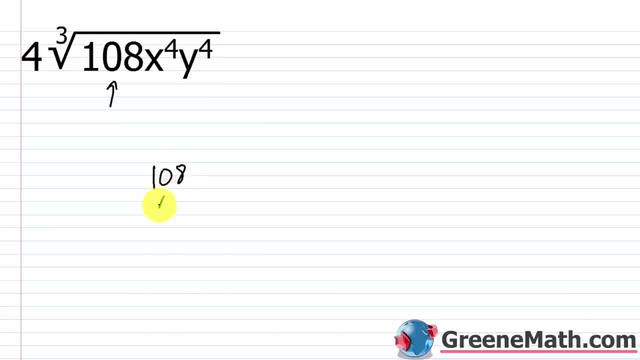 So if I broke down 108, what would I get? So 108 is 27 times 4. 4 is 2 times 2. And then 27 is what? That's a perfect cube. It's 3 times 3 times 3. So let me just kind of stop there. 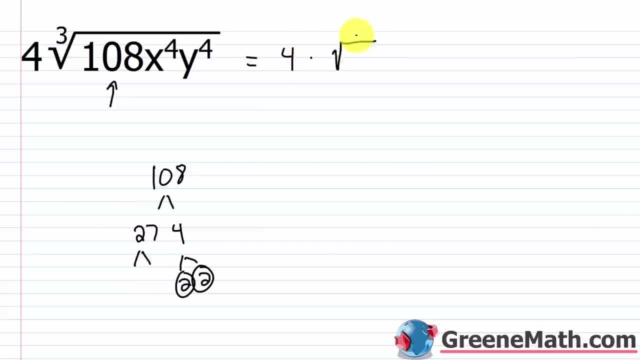 And let me write this as 4 times the cube root of, so 108, I'm going to write 27 here, the cube root of 27, times the cube root of 4. And we can stop there. All right, now I have x to the 4th power, y to the 4th power. Again, what can I do there? To make this easy, think about the 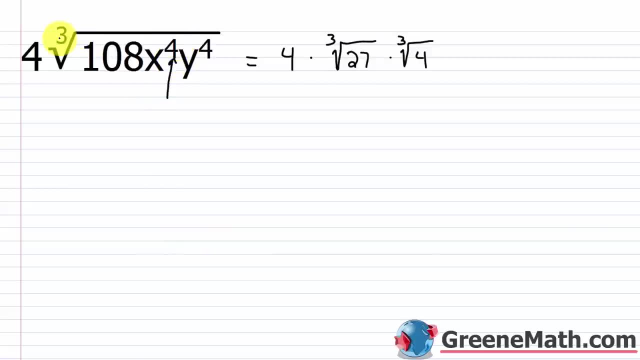 closest number to 4, that's going to be divisible by 3. Well, that's going to be 3, right? So if I add x to the 4th power, y to the 4th power, that's going to be 3. So if I add x to the 4th power, y to the 4th power, y to the 4th power, this right here, the cube root of that is x, right? We talked about that in the last problem. So this right here would say the cube root of x cubed times the cube 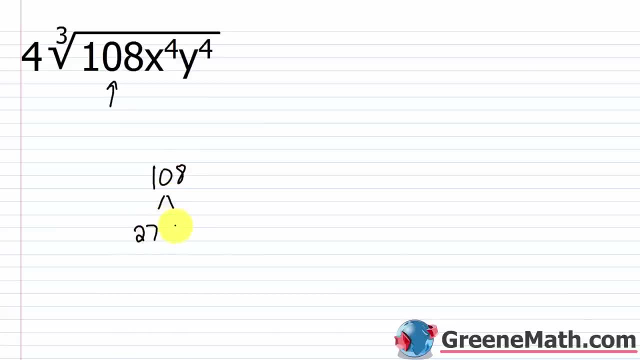 108, what would I get? So 108 is 27 times four, Four is two times two, And then 27 is what? That's a perfect cube. It's three times three times three. So let me just kind of stop there And let me write this as four times the cube root of. 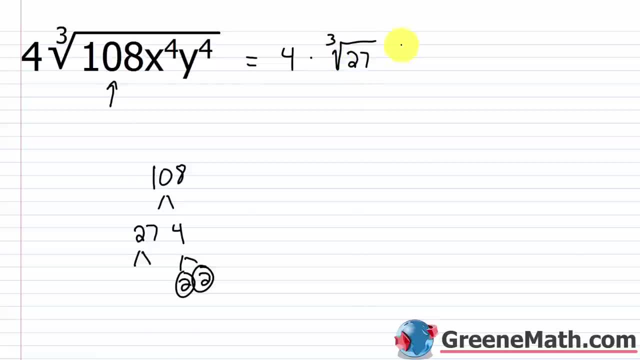 So 108, I'm going to write 27 here, the cube root of 27 times the cube root of four, And we can stop there All right. now I have x to the fourth power, y to the fourth power Again. what can I do there To make this easy? 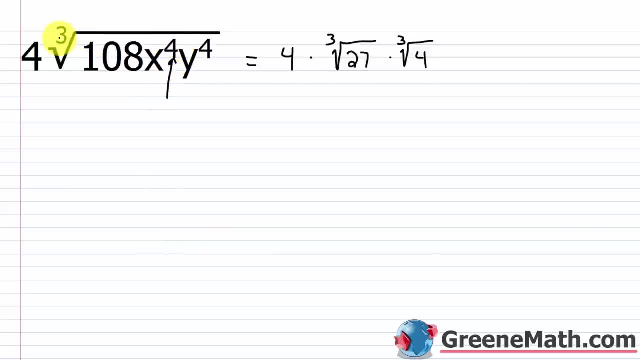 you could say so if I had x to the third power times, x to the fourth power. this right here, the cube root of that is x, right? We talked about that in the last problem. So this right here would say: the cube root of x, cubed times the cube root of x, And then I can. 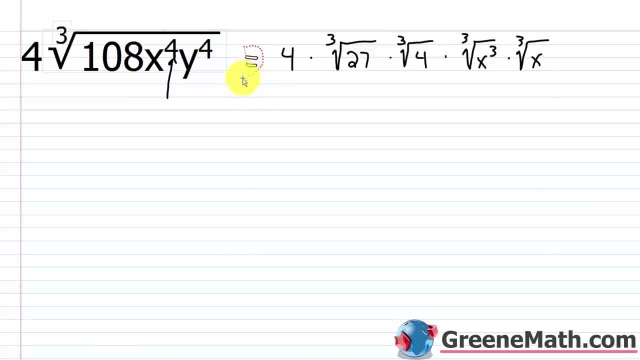 do the same thing for y to the fourth power. Let me kind of scooch all of this down a little bit. So I put times E squared Times x, the cube root of y, cubed times the cube root of y. So you're just breaking these things down to. 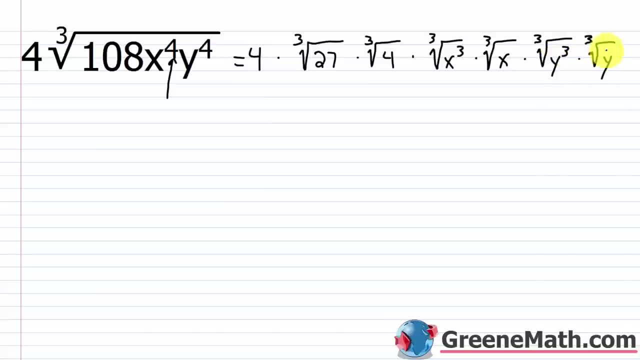 where you're putting in a format where you have a perfect cube and then something that's not going to simplify. So I'm just going to go through. now I have four times the cube root of 27, I know, is three. The cube root of four- let's leave that for a second. The cube root of x cubed I know, is x. 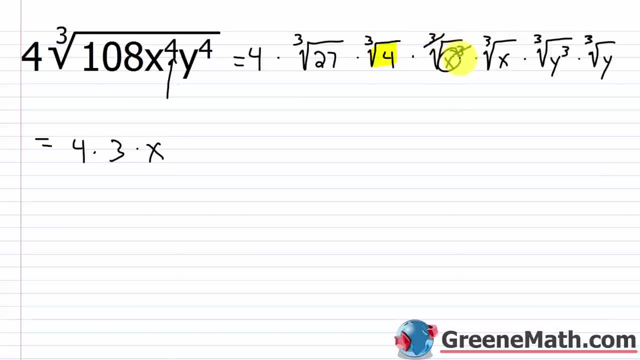 right, Because this would cancel with this and give me this. Then the cube root of x. let's leave that for a minute. The cube root of y cubed is y Again, this would cancel with this and leave me this. And then the cube root of y. let's write this right now. So four times three is 12 times. 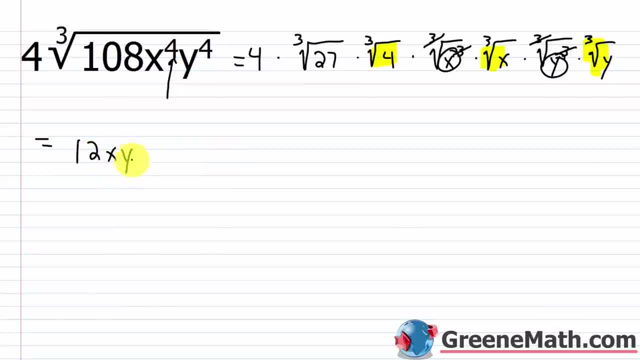 xy. So let's just replace this with 12xy and then times the cube root of. you're going to have a four That can't be simplified, An x that can't be simplified and a y that can't be simplified, So I just write them all under one. 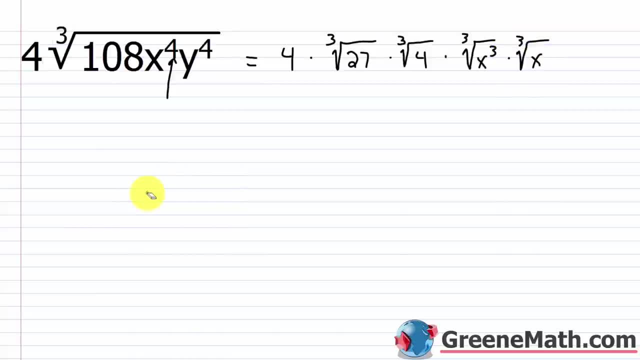 root of x. And then I can do the same thing for y to the 4th power. Let me kind of scooch all this down a little bit. So I put times the cube root of y cubed times the cube root of y. So you're putting things down to where you're putting it in a format where you have a perfect cube and then something that's not going to simplify. So I'm just going to go through now. I have 4 times the cube root of 27 I know is 3. The cube root of 4, let's leave that for a second. The cube root of x cubed I know is x, right? Because this would cancel with this and give me this. Then the cube root of x, let's leave that for a minute. The cube root of y cubed is y. Again, this would cancel with this and leave me this. And then the cube root of y, let's write this right now. So 4 times 3 is 12 times xy. So let's just replace this with 12xy and then times the cube root of. You're going to have a 4 that can't be simplified, an x that can't be simplified, and a y that can't be simplified. So I just write them all under one radical symbol, right? You could spread it out and put cube root of 4 times cube root of x times cube root of y. But really, you don't have to do that. You can just write it. You don't need to do that, right? This is just a more compact way to write it. So 12xy times the cube root of 4xy. All right, let's take a look at one final problem and then we'll wrap up this lesson. So a lot of stuff to take in. And before I kind of do this problem, I want to just 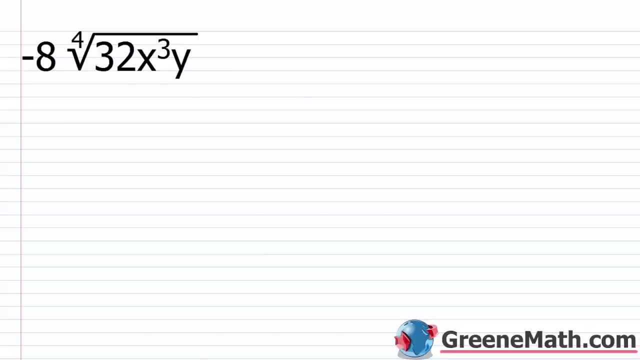 make a little side note. I didn't say this, but another error that students make is they might think something like square root of, let's say, 4 times cube root of, let's say, 8 can be combined, right? I can't. The index in each case has to be the same. This is a 2 and this is a 3. So this is a no-go here. I can't do anything with that. I have to evaluate those separately and say, well, the square root of 4 is 2. The cube root of 8 is 2. So it's 2 times 2 or 4. But I can't, you know, make one radical symbol and say, you know, I've seen students go, okay, well, this is the sixth root of 32, right? That's not going to work. That's wrong, okay? 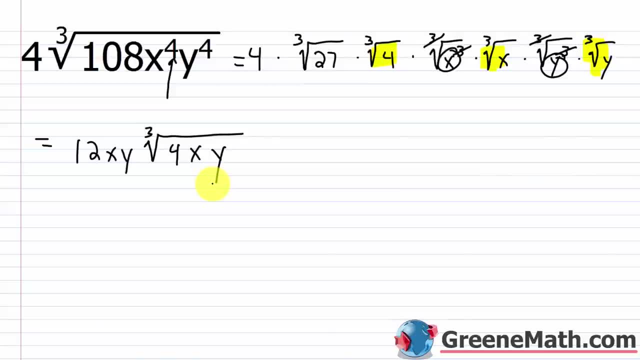 radical symbol, right? You could spread it out and put cube root of four times cube root of x times cube root of y, but really you don't need to do that, right? This is just a more compact way to write it. So 12xy times the cube root of 4xy. All right, let's take a look at one final problem. 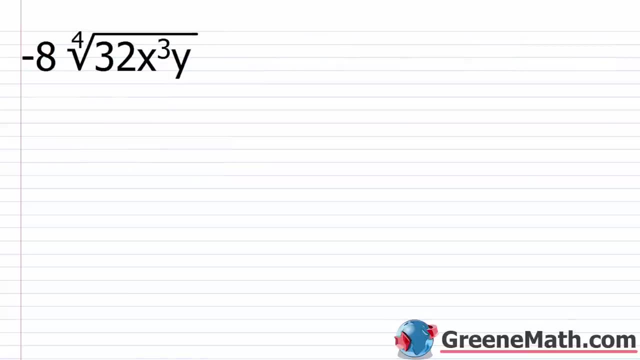 and then we'll wrap up this lesson. So a lot of stuff to take in. And before I kind of do this problem, I want to just make a little side note. I didn't say this, but another error that students make is they might think something like: 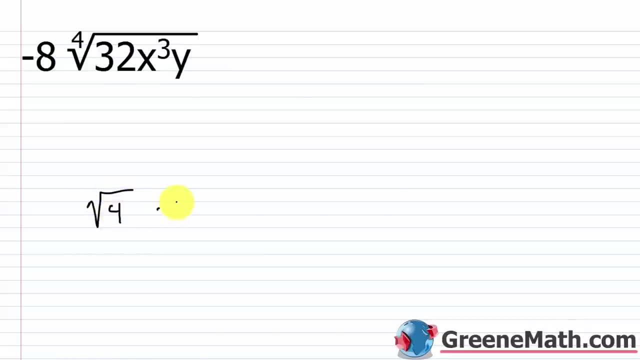 square root of, let's say, four times cube root of, let's say eight, can be combined right? I can't. The index in each case has to be the same. This is a two and this is a three, So this is a no-go here. 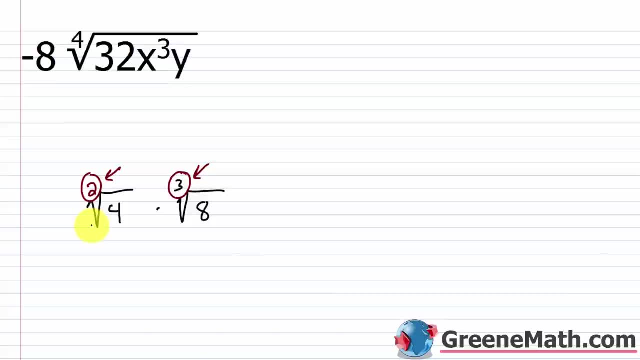 I can't do anything with that. I have to evaluate those separately and say: well, the square root of four is two, The cube root of eight is two, So it's two times two or four, but I can't you know, make one radical symbol and say: 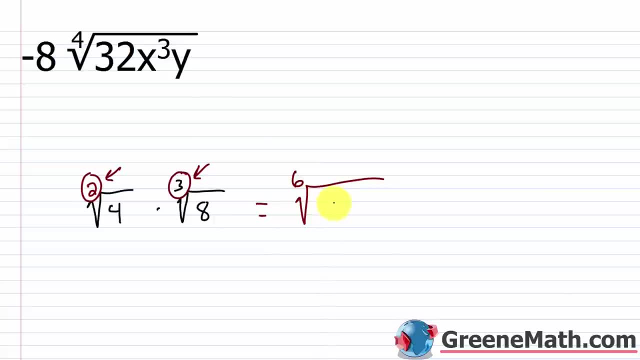 you know, I've seen students go: okay, well, this is the sixth root of 32,. right, That's not going to work, That's wrong. Okay, So another common mistake. All right, So let's tackle this last. 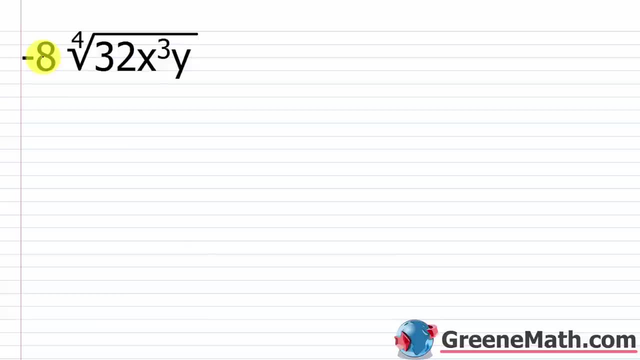 problem here. So we have negative eight times the fourth root of 32x cubed y. So right off the bat we know none of the variables are going to be able to be simplified. How do we know that? Well, if I have the fourth root of something, this would have to at least be. 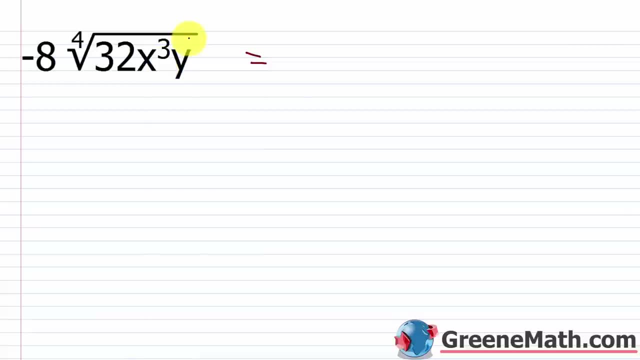 the fourth power for me to pull it outside of the radical symbol. So in my simplified version I know I'm going to have x cubed y, So I can just kind of box those off and forget about it. What can I do with 32? to simplify, 32 is what Four times eight. Eight is four times two And we. 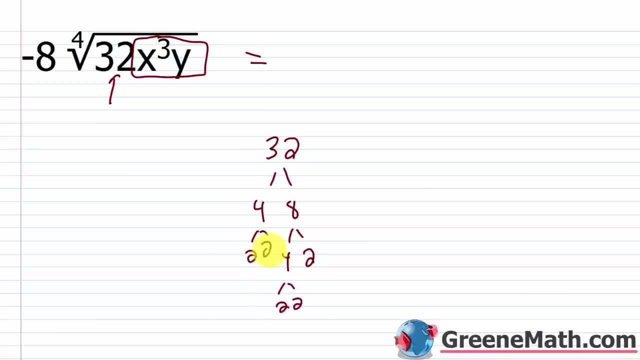 can already see that what This is: two to the fifth power, which I know most of you know that at this point. So it's two to the fourth power times another two right, Or 16 times two. So what I can do here is I can write this as negative: eight times the fourth root of 16 times the fourth root. 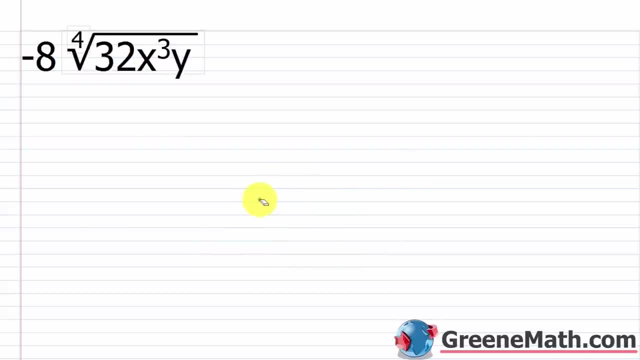 So another common mistake. All right. So let's tackle this last problem here. So we have negative 8 times the fourth root of 32x cubed y. So right off the bat, we know none of the variables are going to be able to be simplified. How do we know that? Well, if I have the fourth root of something, this would have to at least be the fourth power for me to pull it outside of the radical symbol. So in my simplified version, I know I'm going to have x, cubed y. So I can just kind of box those off and forget about it. What can I do with 32 to simplify? 32 is what? 4 times 8. 8 is 4 times 2. And we can already see that what? This is 2 to the fifth power, which I know most of you know that at this point. So it's 2 to the fourth power times 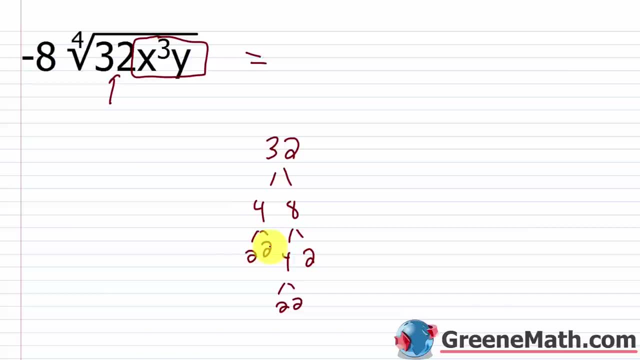 another 2, right? Or 16 times 2. So what I can do here is I can write this as negative 8 times the fourth root of 16. 16 times the fourth root of 2 times x cubed times y. So everything else that's not going to simplify. And then it's very, very simple, right? The fourth root of 16 is 2. So I put equals negative 8 times the fourth root of 16 is 2. We can go ahead and just simplify that now. Negative 8 times 2 is negative 16. And then times the fourth root, the fourth root of 2x cubed y. 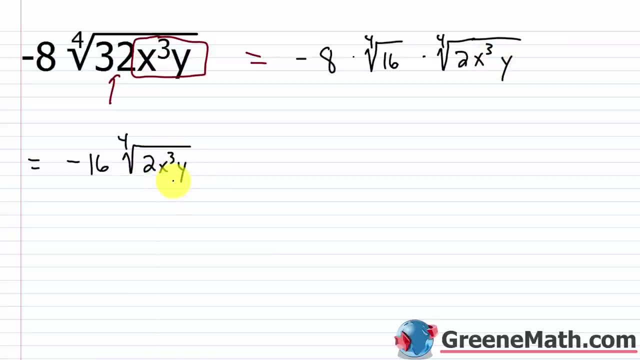 2x cubed y. And there's nothing else to simplify here, right? So that's just your answer. Negative 16 times the fourth root of 2x cubed y. Hello, and welcome to Algebra 1, Lesson 55. In this video, 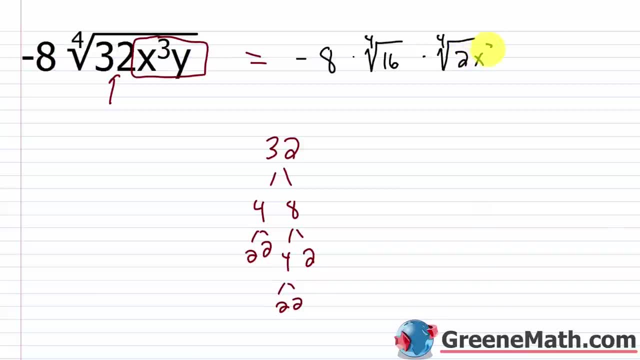 of two times x cubed times y. So everything else that's not going to simplify. And then it's very, very simple, right? The fourth root of 16 is two. So I put: equals negative eight times the fourth root of 16 is two. We can go ahead and just simplify that. now. Negative eight times two is 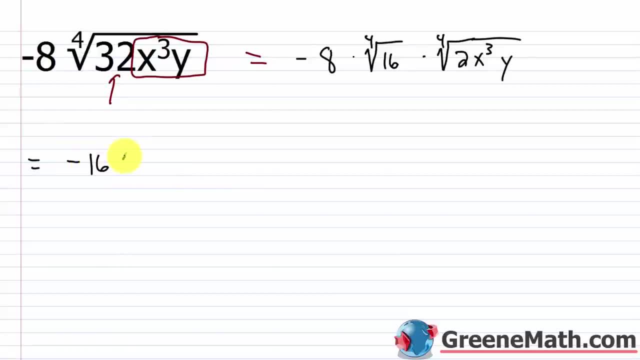 negative 16.. And then times the fourth root, the fourth root of two x cubed y, two x cubed y- And there's nothing else to simplify here, right? So that's just your answer: Negative 16 times the fourth root of two x cubed y. Hello and welcome to Algebra 1, Lesson 55.. In this video we're going: 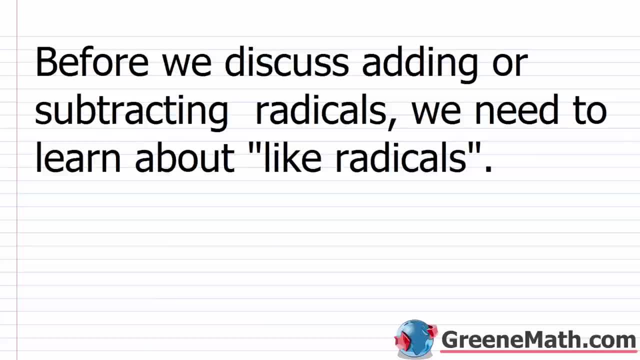 to talk about radicals. So before we discuss adding or subtracting radicals, we need to learn about something known as like radicals. And before I even tell you about like radicals, I want to kind of just remind you that we saw something like this already, So I want you to recall when we first 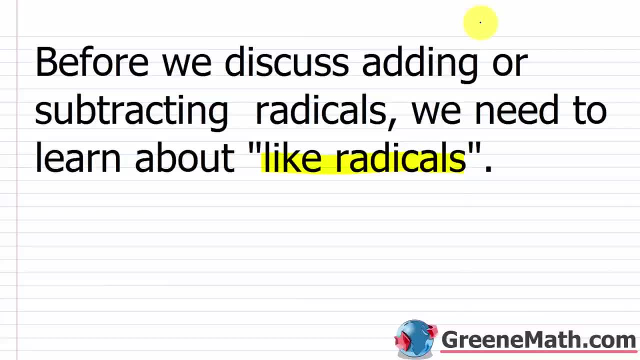 started working with terms. we talked about something known as like terms, right? So in the case of a single variable, like terms would be the same variable raised to the same power. So, in other words, if I had three x and I had five x, those were like terms, But if I had something, 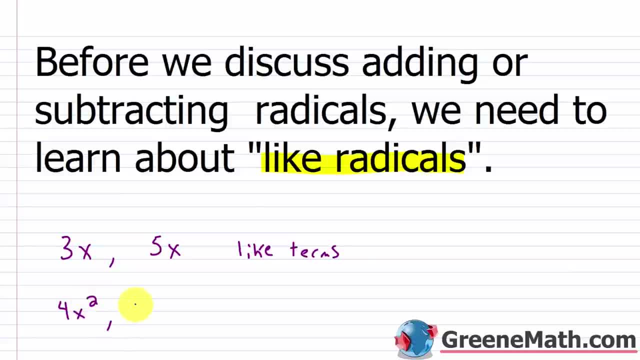 like, let's say, four x squared and I had five x cubed. those were not like terms. Those were not like terms, And why? Because you had to have the same variable, which, in this case, you have the same variable. In this case, you have the same variable. But the kicker to that is: 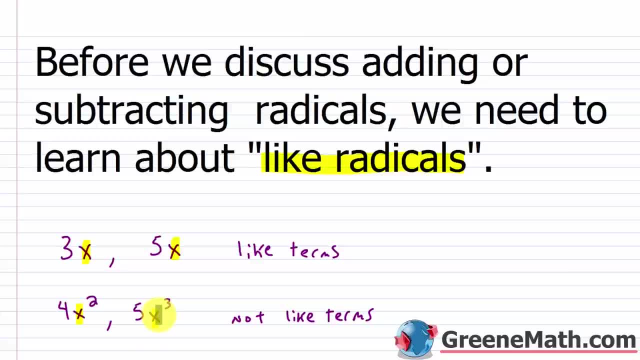 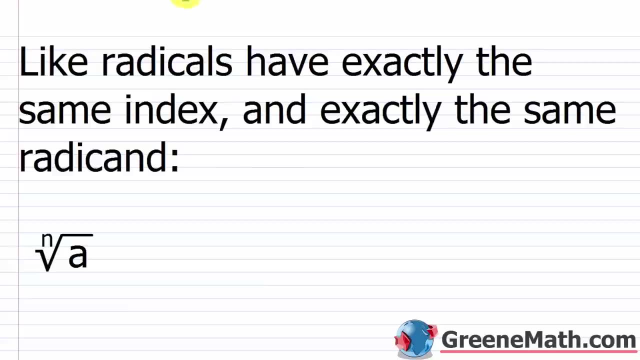 you also have to have the same exponential power And in this particular case you have a two here and a three here, So they're not like terms. So again, similar to this, we have like radicals, So like radicals have exactly the same index. So exactly the same index and exactly the same. 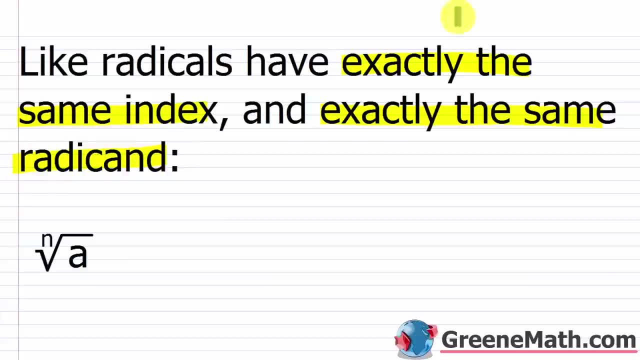 radicand. So in case you forgot the terminology, this right here is your index. so this is your index And I know a lot of times we work with square roots And when you see a square root- let's say you had square root of four- the index is left blank, right, But really. 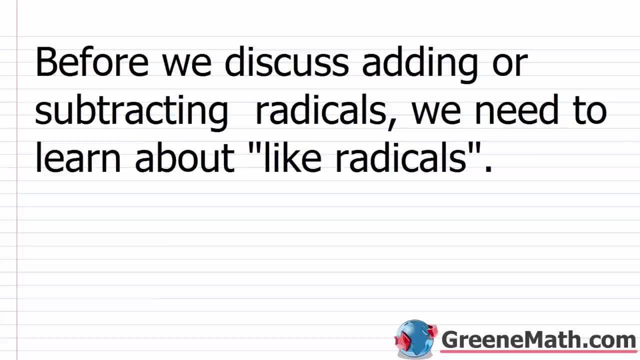 we're going to learn about adding and subtracting radicals. So before we discuss adding or subtracting radicals, we need to learn about something known as like radicals. And before I even tell you about like radicals, I want to kind of just remind you that there's a lot of things that we saw something like this already. So I want you to recall when we first started working with terms, we talked about something known as like terms, right? So in the case of a single variable, like terms would be the same variable raised to the same power. So in other words, if I had 3x and I had 5x, those were like terms. But if I had something like, let's say, 4x squared, 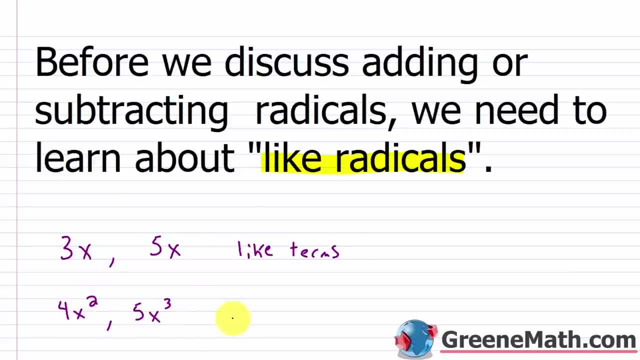 and I had 5x cubed, those were not like terms. Those were not like terms. And why? Because you had to have the same variable, which in this case, you have the same variable. In this case, you have the same variable. But the kicker to that is you also have to have the same exponential power. And in this particular case, you have a 2 here and a 3 here. So they're not like terms. So again, similar to this, 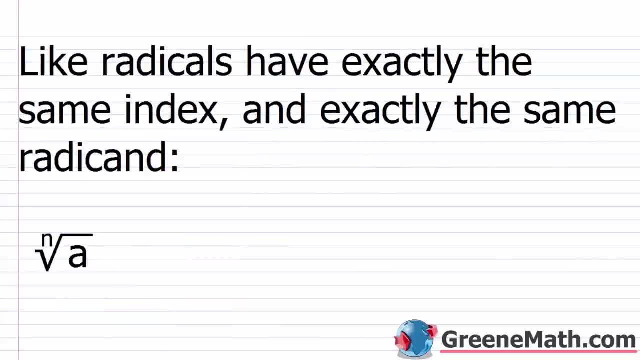 you have like radicals. So like radicals have exactly the same index. So exactly the same index and exactly the same radicand. So in case you forgot the terminology, this right here is your index. So this is your index. And I know a lot of times we work with square roots. And when you see a square root, let's say you had a square root of 4, the index is left blank, right? But really, the index is left blank. So this is your index. And I know a lot of times we work with square roots. And I know a lot of times we work with square roots. And I know a lot of times we work with a 2. Just with square roots, because they're so common, we just leave it blank. And it's understood to be a 2. So this is your index. I'm just going to write a 2 in right there. 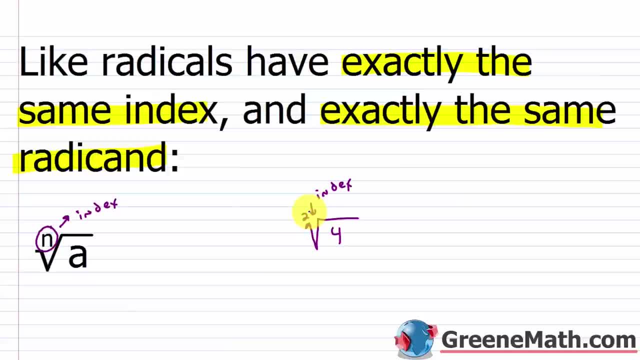 Now, the number, or it could be the variable that's underneath your radical symbol is known as a radicand. So in this case, the a would be called the radicand. 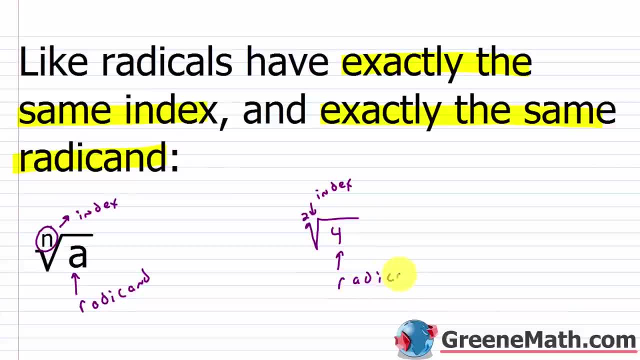 So this would be the radicand. And then you have the index. And I know a lot of times we work with be the radicand. So for us, again, to have like radicals, we have to have the same index and the 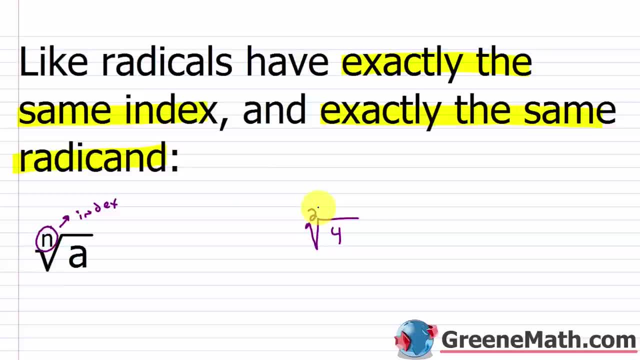 the index is a two, just with square roots, because they're so common. we just leave it blank and it's understood to be a two. So this is your index. I'm just going to write a two in right there Now the number, or it could be the variable. 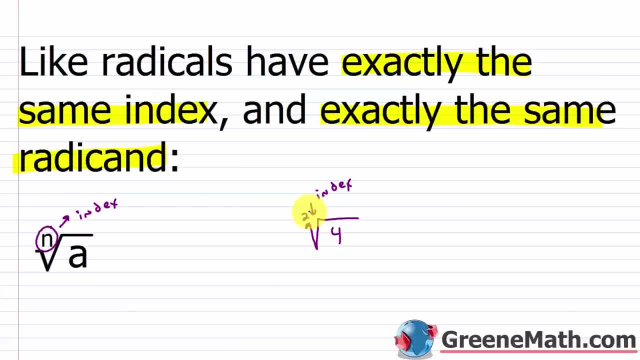 that's underneath your radical symbol is known as a radicand. So in this case the A would be called the radicand. So this would be the radicand. So for us again to have, like radicals we have to. 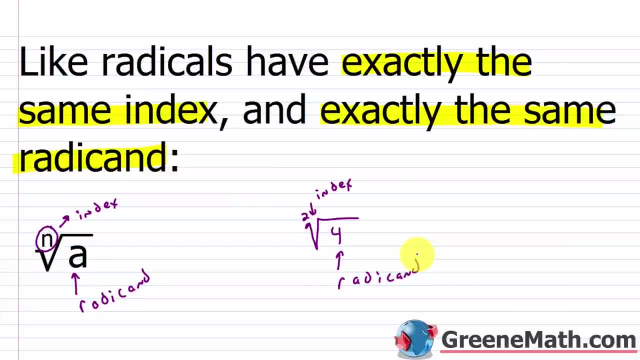 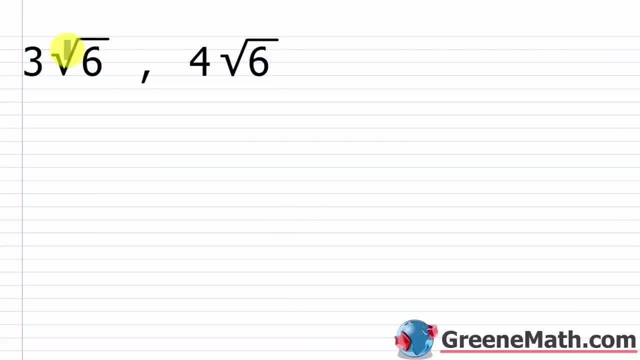 have the same index and the same radicand. So that's what we're going to be looking for, All right, so in this first example here, I'm going to look at the index. in this case, it's going to be a two here and a two here, right, If you don't see anything? 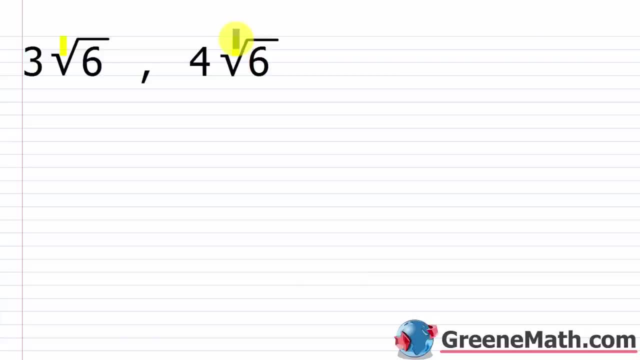 it's understood to be a two, because we recognize this as a square root. Then I'm looking at the radicand: In this case it's the six And in this case it's a six, So we have the same. 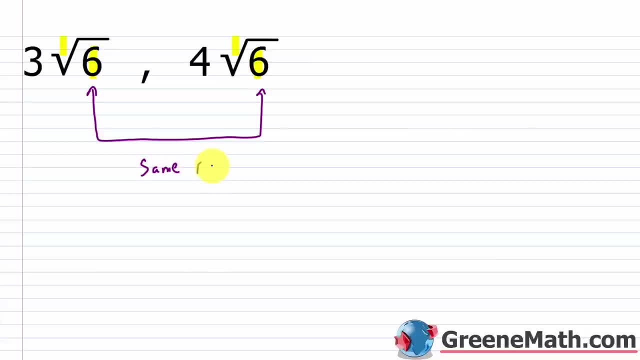 right, the same radicand, And then we also have the same, the same index. So these would be like radicals. These are like radicals. What about something like 7 times square root of 9 and 2 times the cube root of 9?? Well, these are not like radicals. Although the radicand 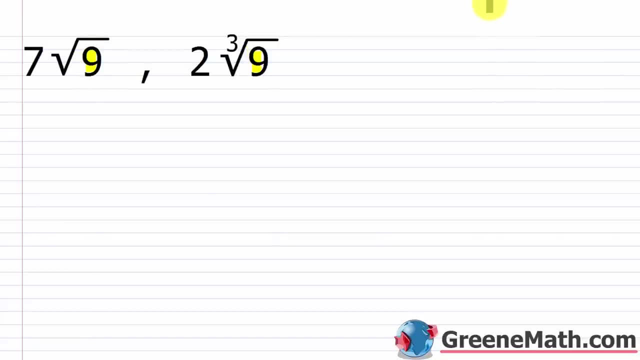 is the same in each case. this is a 9 and this is a 9,. you'll notice that your index here is a 3 and then your index here is a 2, right? If you don't have an index, you can write in a 2 or just. 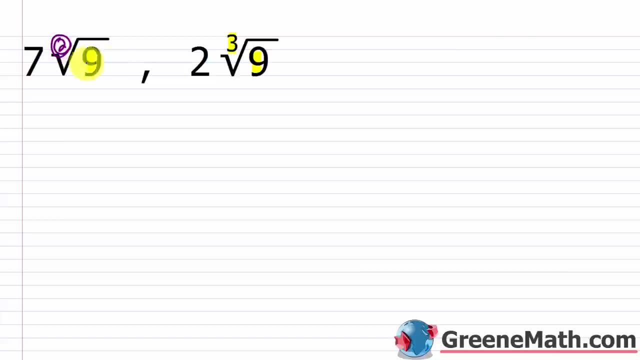 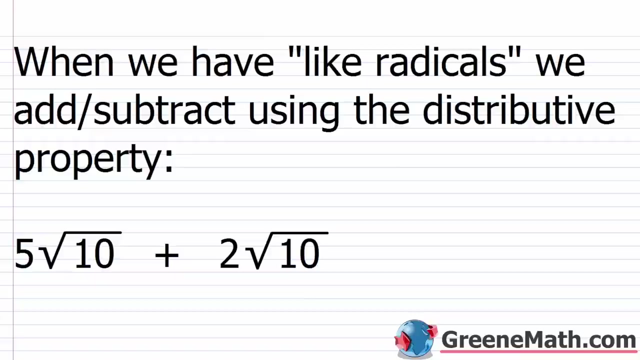 understand that it's a 2. It's for a square root right, So the indexes are not the same in this case. So these are not like radicals, So not like radicals, All right. so pretty easy overall to understand if you have a like radical or not a like radical. Again, I always explain this with: 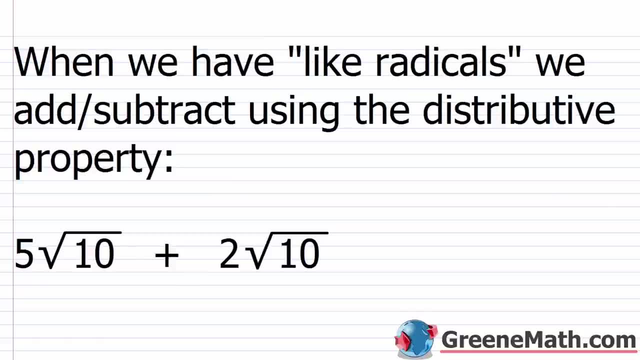 that concept of like terms because essentially it's the same level of understanding. Once you figured out what like terms were, it was very, very easy to combine them right, Using the distributive property. So when we talk about like radicals, it's going to be the same thing. 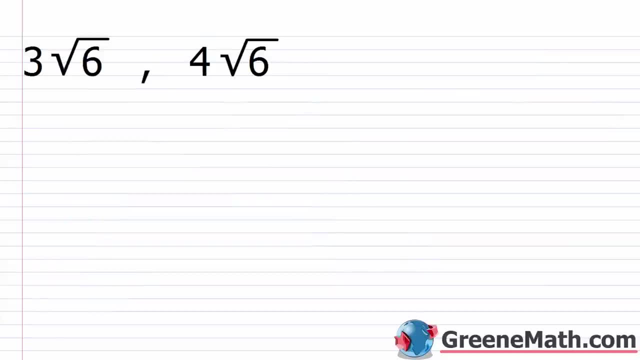 same radicand. So that's what we're going to be looking for. All right, so in this first example here, I'm going to look at the index. In this case, it's going to be a 2 here and a 2 here, right? If you don't see anything, it's understood to be a 2 because we recognize this as a square root. Then I'm looking at the radicand. In this case, it's a 6, and in this case, it's a 6. So we have the same, right, the same radicand, and then we also have the same index. 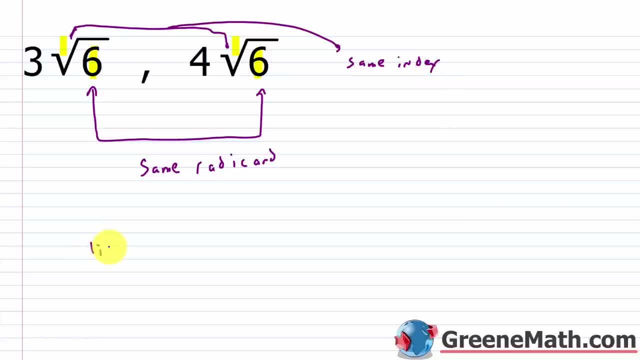 So these would be like radicals. These are like radicals. 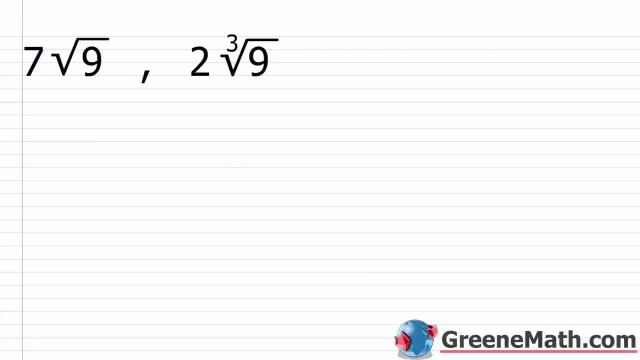 What about something like 7 times square root of 9 and 2 times the cube root of 9? Well, these are not like radicals. Although the radicand is the same in each case, this is a 9 and this is a 9, you'll notice that your index here is a 3, and then your index here is a 2, right? If you don't have an index, you can write in a 2 or just understand that it's a 2. It's for a square root, right? So the indexes are not the same in this case, so these are not like radicals. So not like radicals. All right, so pretty easy overall to understand if you have a like radical or not 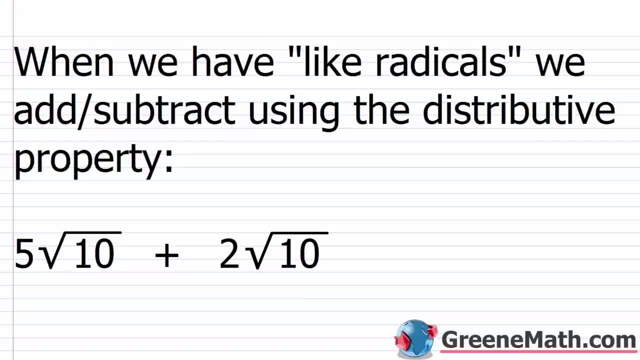 a like radical. Again, I always explain this with that concept of like terms because essentially, it's the same level of understanding. Once you figured out what like terms were, it was very, very easy to combine them, right, using the distributive property. 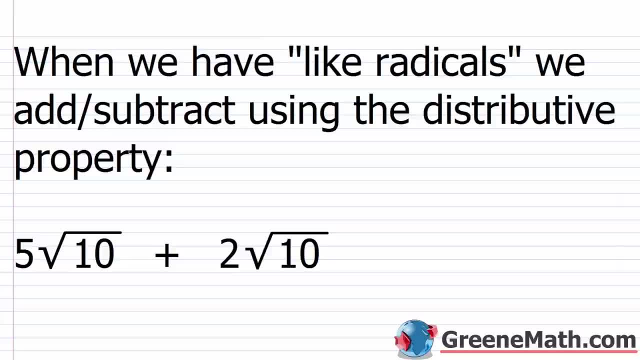 So when we talk about like radicals, it's going to be the same thing. It's going to be very, very easy to combine them using your distributive property. 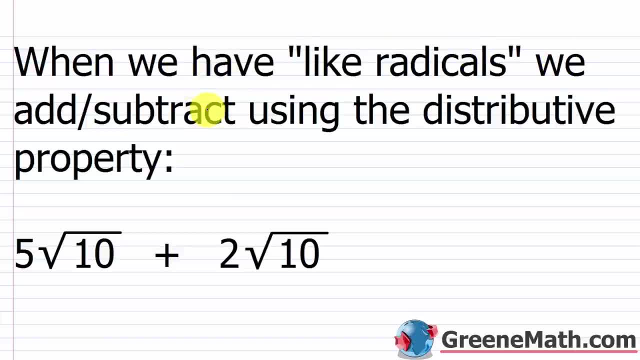 So when we have like radicals, we add or subtract using the distributive property. 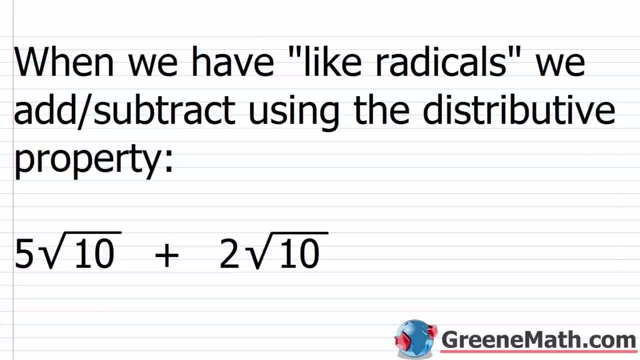 It's going to be very, very easy to combine them using your distributive property. So when we have like radicals, we add or subtract using the distributive property. Now, before I even do this example, let me just show you real quick with something that you already know. If I had, 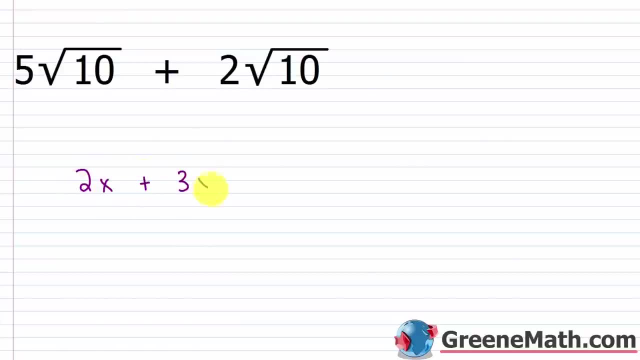 something like 2x plus 3x. I know that that's 5x, But at this point we might have forgotten that we started out with a 5x. So we're going to start out with a 5x And we're going to start out with. 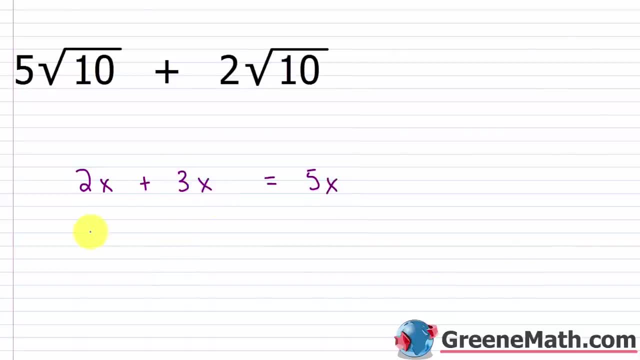 by saying that we could factor an x out and write this as x times a quantity: 2 plus 3, right, Because x was common to each. So if I factored it out, I'd have a 2 left here and a 3 left here, So that's. 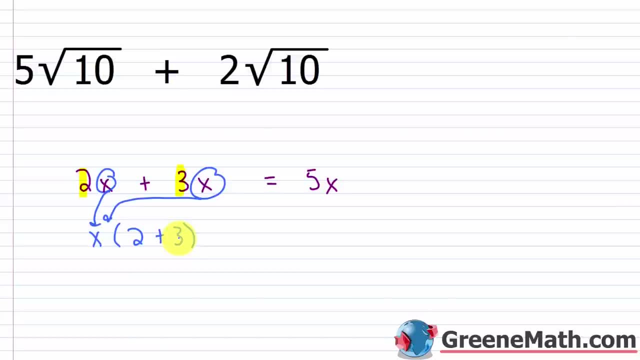 where I got this 2 plus 3.. Now if I did that operation- 2 plus 3, I'd get 5. And I'd be multiplying by x so I get 5x. So we kind of shorten this process up by saying: okay, I know that the x is. 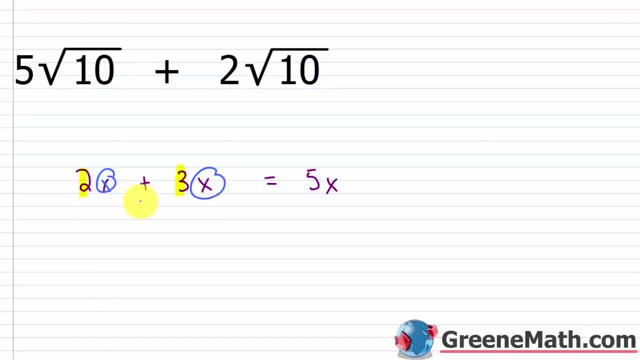 common to each of these. So really all I need to do is add the coefficients and then slap an x at the end. So I would say 2 plus 3 is 5, slap an x at the end, I get 5x. Or if I was adding something. 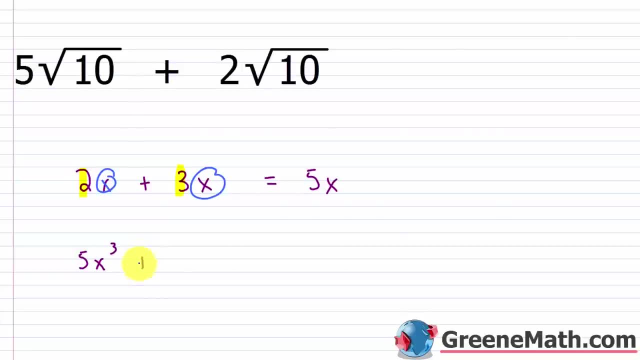 like, let's say, 5x cubed plus 7x cubed. I know these are like terms. the x cubed is just going to be there, right? Same variable raised to the same power. that's going to be there, I just add. 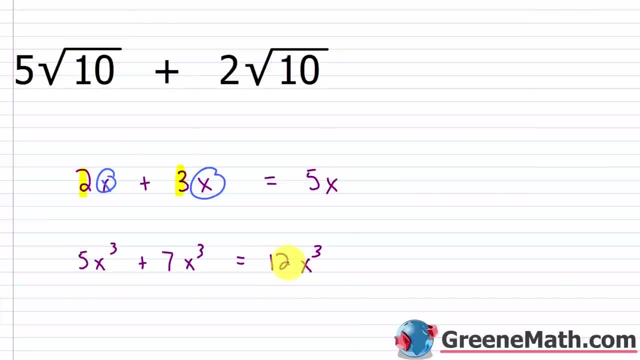 the coefficients. So 5 plus 7 is 12.. So I have 12x cubed. So we already know how to execute that process and it's basically going to be the exact same thing with radicals. So if I look at this first example here, a lot of you can. 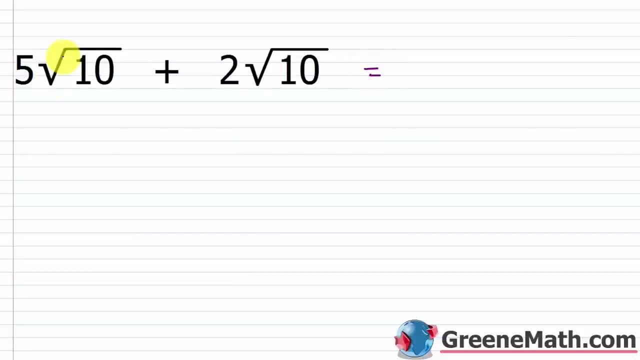 kind of guess what to do. So I have 5 times the square root of 10 plus 2 times the square root of 10.. So the first thing you do is check to make sure that you have like radicals. So we have the. 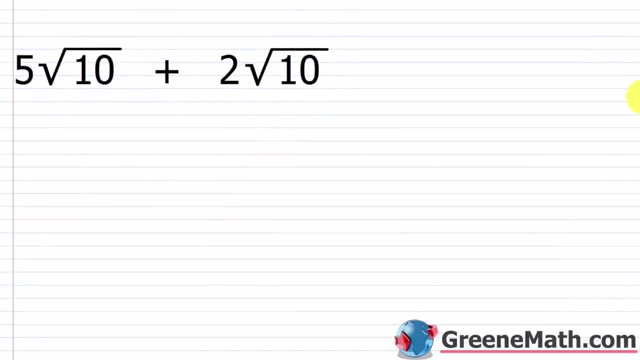 Now, before I even do this example, let me just show you real quick with something that you already know. If I had something like 2x plus 3x, I know that that's 5x. But at this point, we might have forgotten that we started out by saying that we could factor an x out and write this as x times a quantity 2 plus 3, right? Because x was common, but in reality, we would have needed to write x to add theят dashed until the firstnost to the end of the picture. So we could now do the same thing to what we did to before. The same is sorted by架 saying like, because 2 plus 3 is falling in, so I'm going to write 2 plus 3 dash ?? to each. So if I factored it out, I'd have a two left here and a three left here. So that's where I got this two plus three. 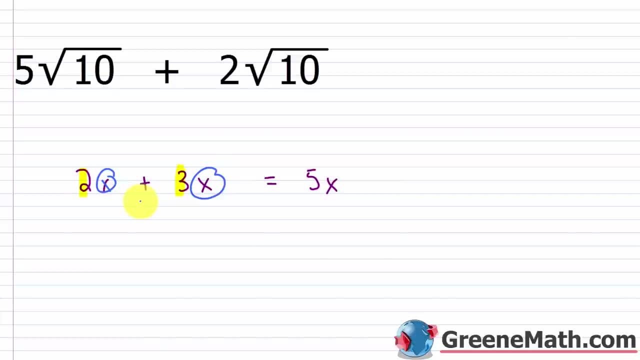 So I would say 2 plus 3 is 5, slap an X at the end, I get 5X. Or if I was adding something like, let's say 5X cubed plus 7X cubed, I know these are like terms, the X cubed is just going to be there, right? Same variable, raised to the same power, that's going to be there. I just add the coefficients. 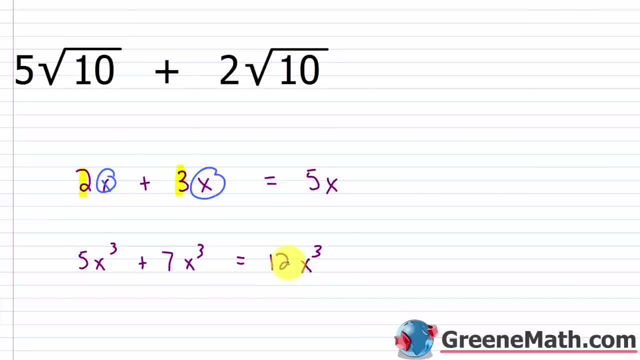 So 5 plus 7 is 12, so I have 12X cubed. So we already know how to execute that process, 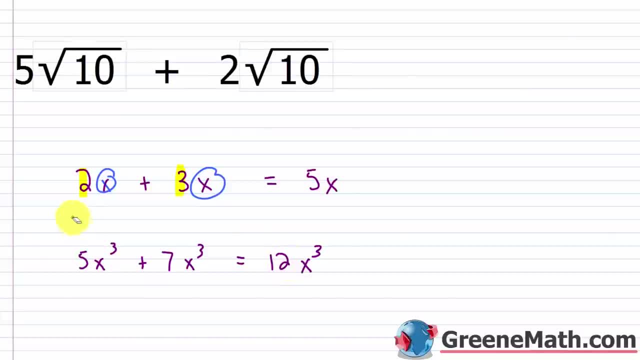 and it's basically going to be the exact same thing with radicals. So if I look at this first example here, a lot of you can kind of guess what to do. 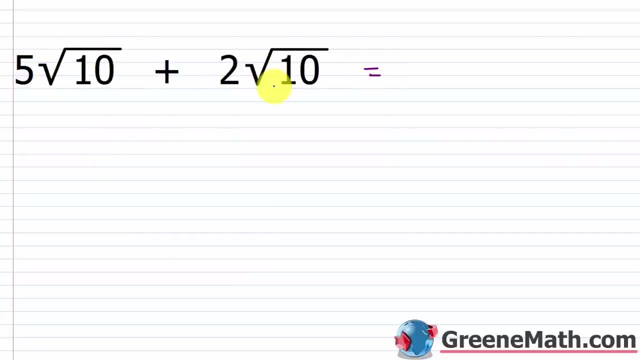 So I have 5 times the square root of 10 plus 2 times the square root of 10. 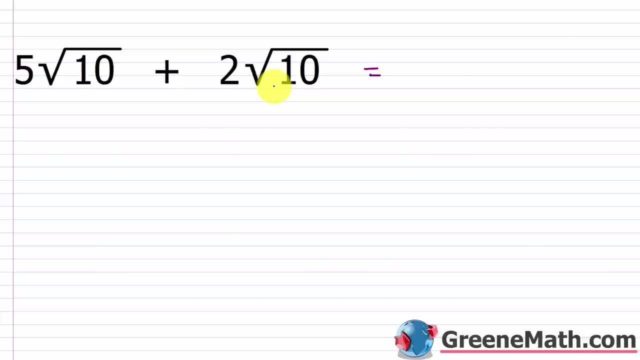 So the first thing you do is check to make sure that you have like radicals. So we have the same index, they're both square roots, and then we have the same radicand. This is a 10, and this is a 10. So we're good to go there. 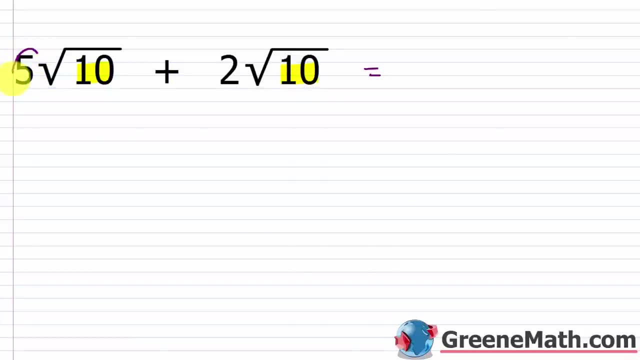 So essentially all I'm going to do is add the numbers out of the square root of 10 to the square root of 10. So 5 plus 2 would give me 7, and then it's times that common square root of 10. 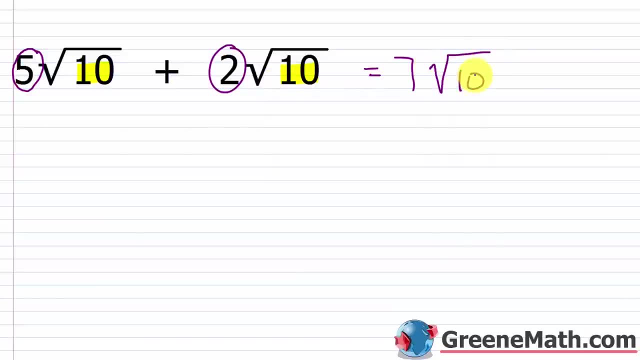 So 7 times the square root of 10. You just think of it as I have 5 times some quantity plus 2 of the same quantity. That gives me 7 of that quantity, and that quantity is the square root of 10. 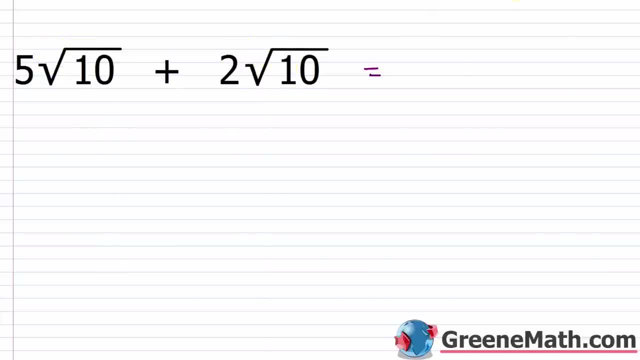 same index. they're both square roots. and then we have the same radicand. This is a 10, and this is a 10.. So we're good to go there. So, essentially, all I'm going to do is add the numbers outside here. So 5 plus 2 would give me. 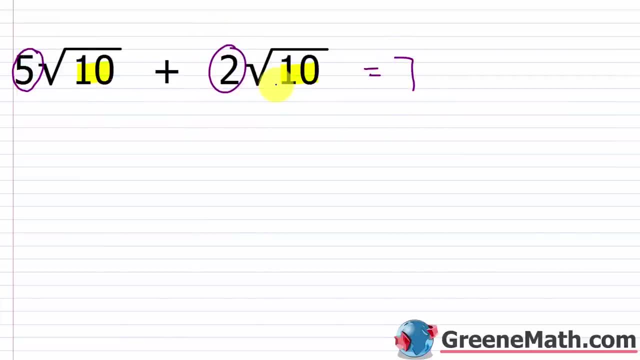 7, and then it's times that common square root of 10.. So 7 times the square root of 10.. You just think of it as I have 5 times some quantity plus 2 of the same quantity, That gives me 7 of that. 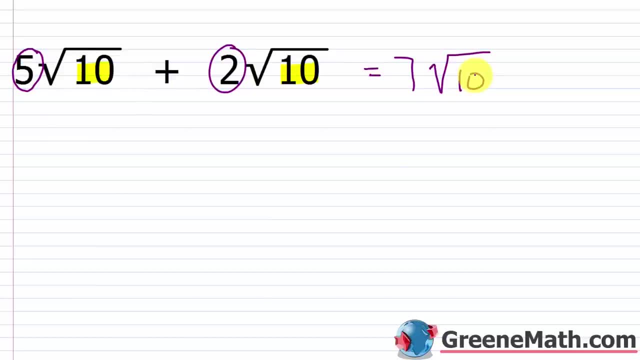 quantity, and that quantity is the square root of 10,, right? If I had 5x plus 2x, this would be 7x, right? It's no different what we're doing here, And if you wanted to use your factoring that, you've. 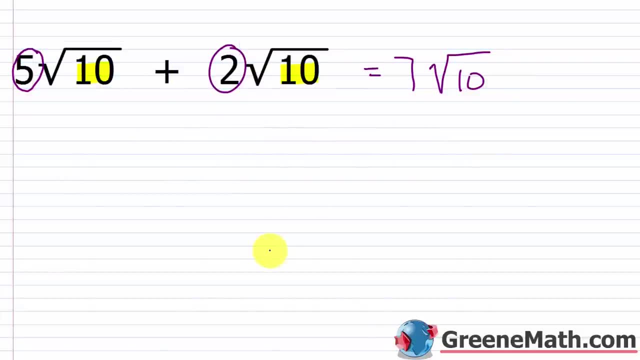 learned to this point. to completely break it down, you could do that as well. I have a square root of 10. that's common to both, so I could factor that out. I would have the square root of 10, and then, inside of parentheses, I'd have a 5 plus a 2.. Now, what does this equal? Well, I have square root of. 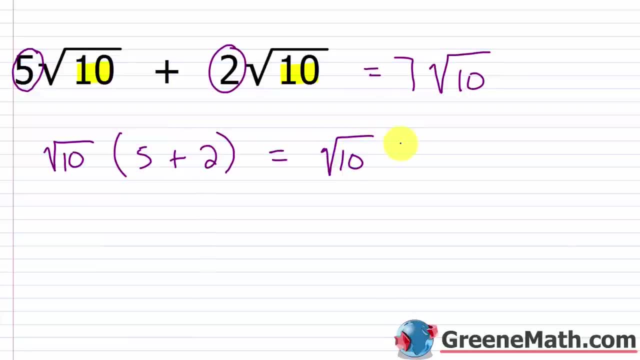 10 times 5 plus 2 is 7.. So times 7, and I could rearrange that and write 7 times 7.. So I could write 7 times square root of 10, like that. So whatever you need to do to make this make sense, 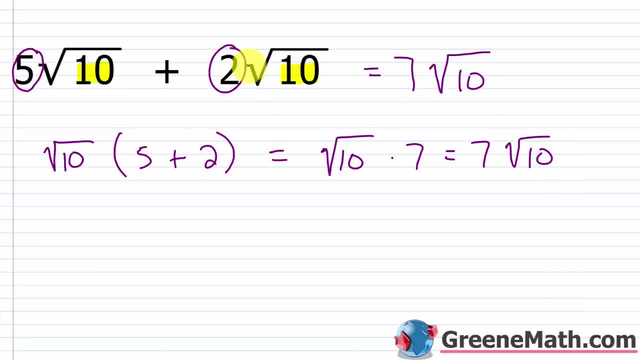 for you. Again, the easiest way to do it is just to think about what's outside of your radical symbol. You're adding those together or subtracting them, depending on your operation that you're performing, And then what's common here in this case is square root of 10.. It's just coming along for. 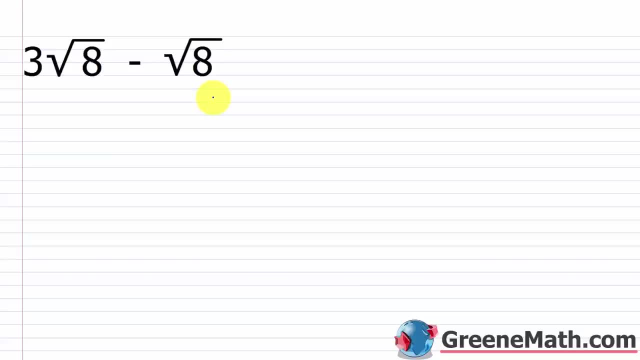 the ride. So what about something like 3 times the square root of 8 minus the square root of 8?? Well, the first thing is to realize: remember, if we saw something like minus x, we would say, okay, there's no coefficient for x, so it's understood to be 1.. 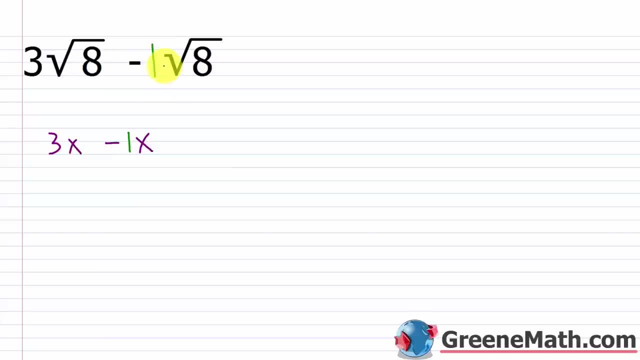 Well, it's kind of the same thing here. We have an understood 1, that's multiplying that square root of 8.. So if I go to perform this operation here, all I need to do is think about the numbers in front: So 3, and then we can think about that as negative 1.. So 3 minus 1 would be 2,. 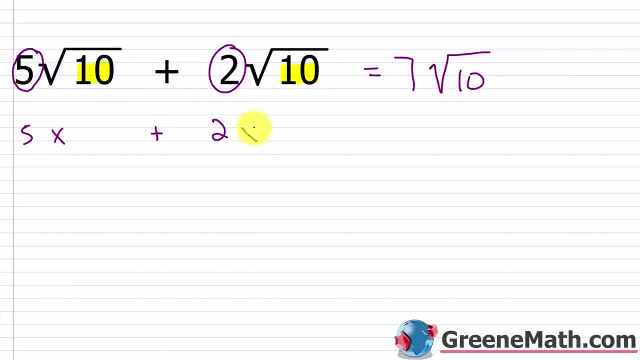 If I had 5X plus 2X, this would be 7X. 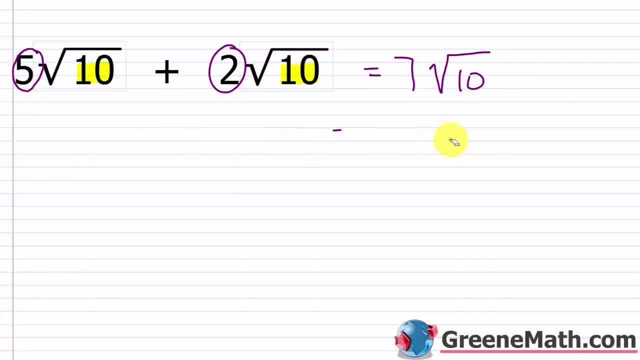 It's no different what we're doing here. And if you wanted to use the square root of 10, 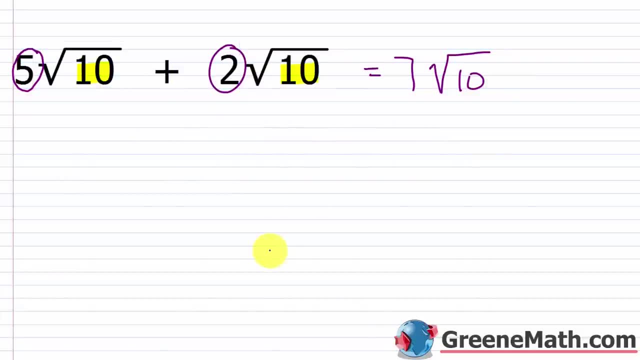 if you wanted to use your factoring that you've learned to this point to completely break it down, you could do that as well. 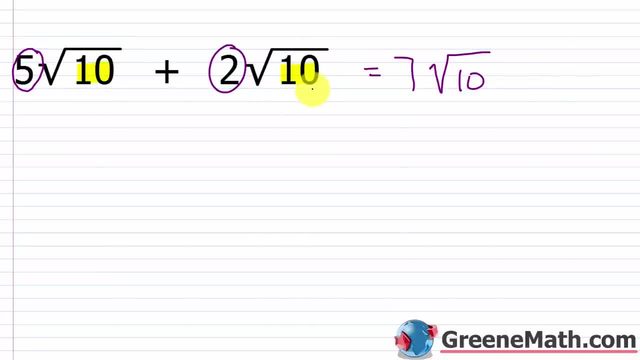 I have a square root of 10 that's common to both, so I could factor that out. I would have the square root of 10, 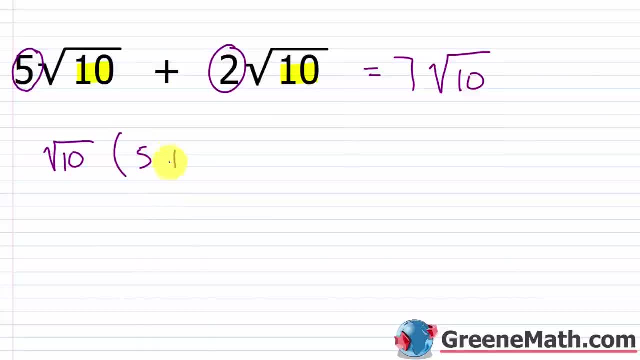 and then inside of parentheses I'd have a 5 plus a 2. Now what does this equal? Well, I have square root of 10 times 5 plus 2 is 7. 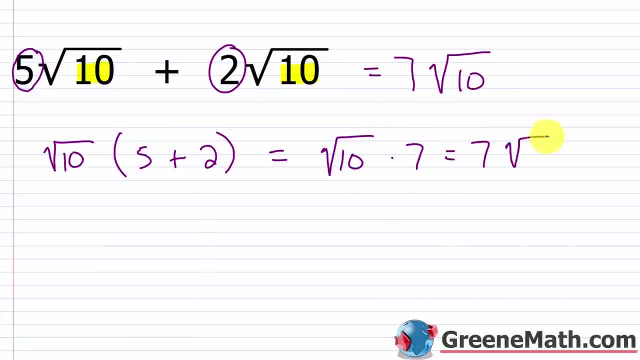 So times 7, and I could rearrange that and write 7 times square root of 10 like that. So whatever you need to do to make this make sense for you. 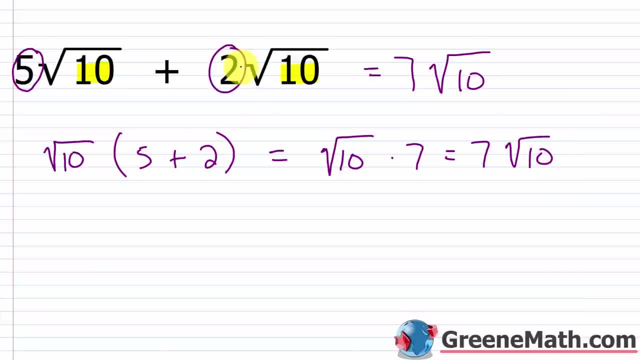 Again, the easiest way to do it is just to think about what's outside of your radical symbol. 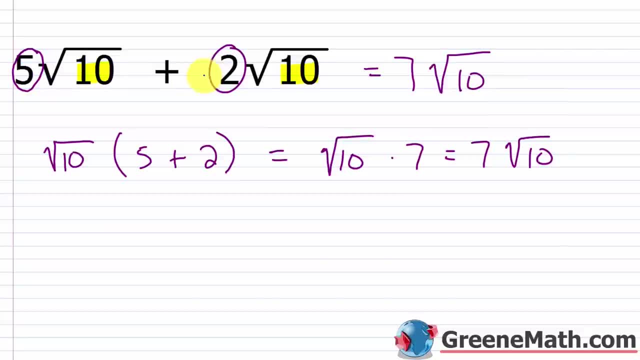 You're adding those together or subtracting them depending on your operation that you're performing. 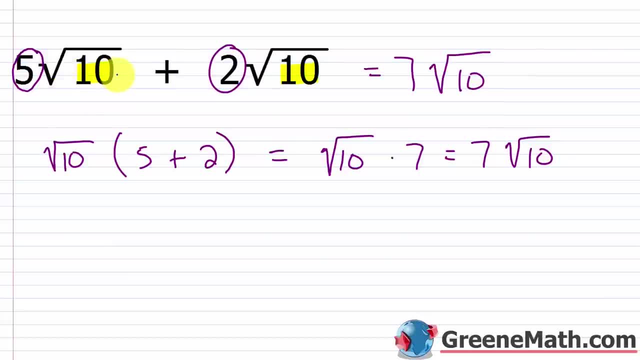 And then what's common here, in this case is square root of 10, is just coming along for the ride. So what about something like 3 times the square root of 8 minus the square root of 8? 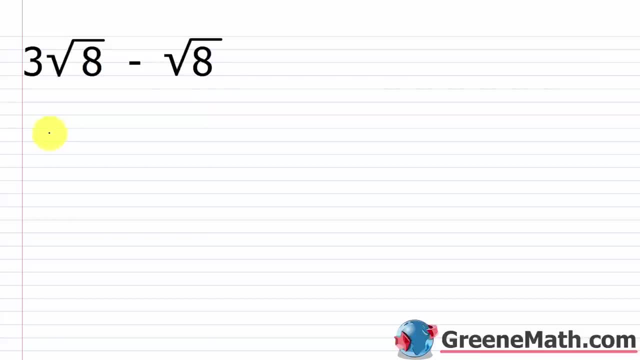 Well, the first thing is to realize, remember if we saw something like 3X minus X, we would say, okay, there's no coefficient for X, so it's understood to be 1. 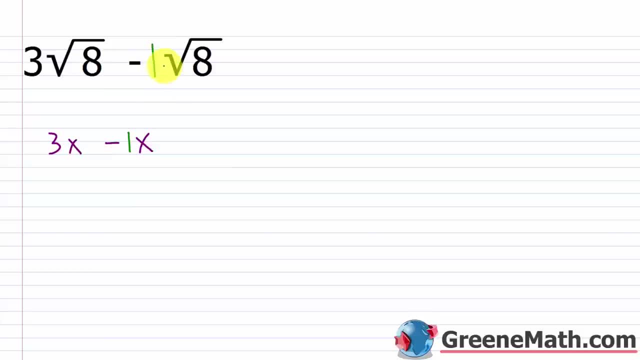 Well, it's kind of the same thing here. We have an understood 1 that's multiplying that square root of 8. So if I go to perform this operation here, all I need to do is think about the numbers in front, so 3, and then we can think about that as negative 1. So 3 minus 1 would be 2, and then times the square root of 8. Now, are we good to go if we leave our answer like this? No, we're not. Right? We learned in the last, 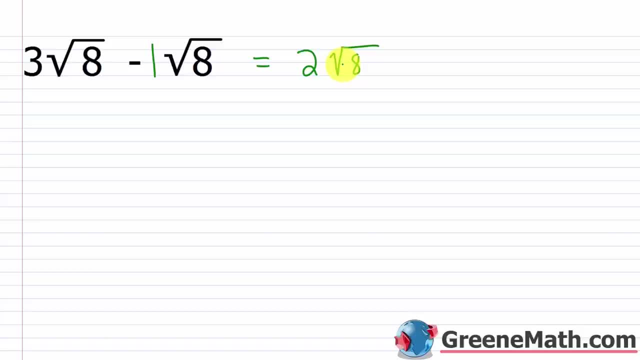 last lesson that we can simplify our radicals. 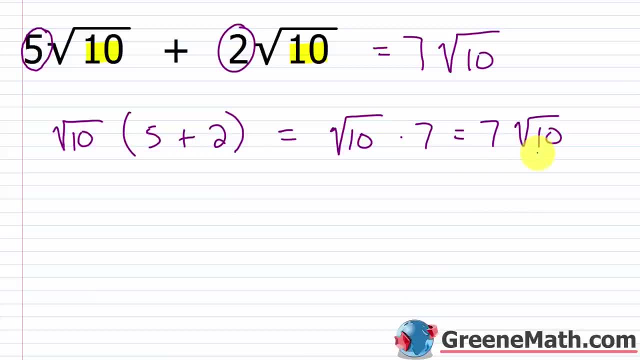 So in the previous example, we ended up with an answer of 7 times the square root of 10. I can't simplify that any further 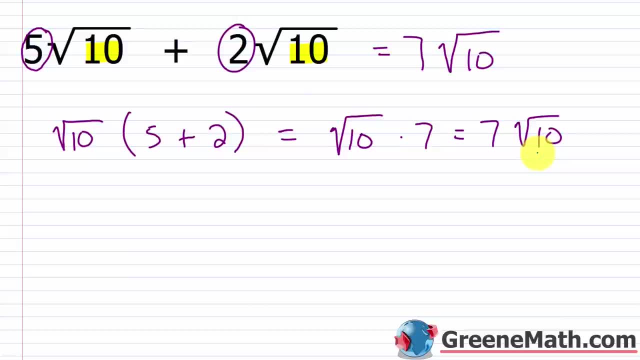 because what's underneath that radical symbol, a 10 is 5 times 2. There's no perfect square underneath there 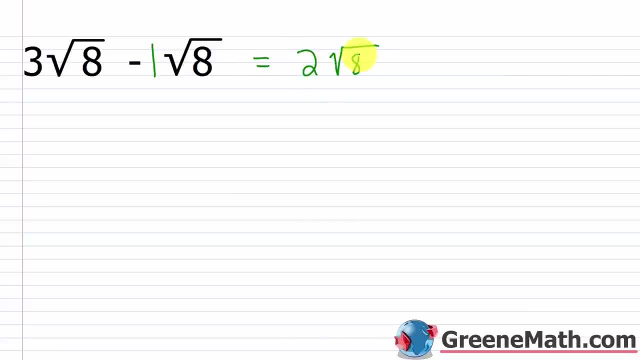 and then times the square root of 8.. Now are we good to go if we leave our answer like this? No, we're not right. We learned in the last lesson that we can simplify our radicals, So in the previous example, we ended up with an answer of 7 times the square. 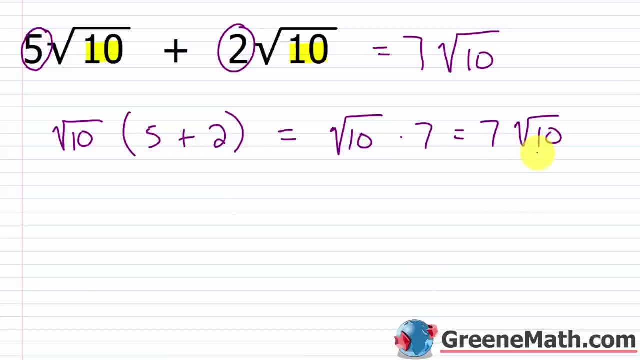 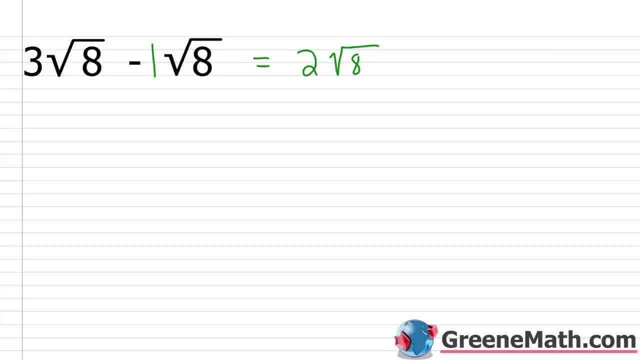 root of 10.. I can't simplify that any further, because what's underneath that radical symbol? a 10 is 5 times 2.. There's no perfect square underneath there that I can kind of work with, So I've got to leave it in that format. In this example, if I factored 8, I could make it 4 times. 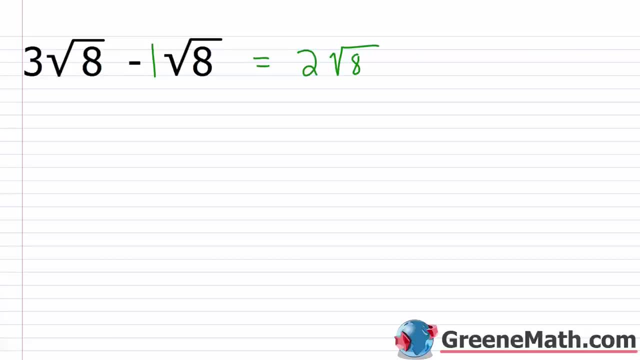 2.. 4 is a perfect square, so I've got to get that out of there. So let's rewrite this as 2 times square root of 4 times square root of 2.. I know the square root of 4 is 2, so essentially what? 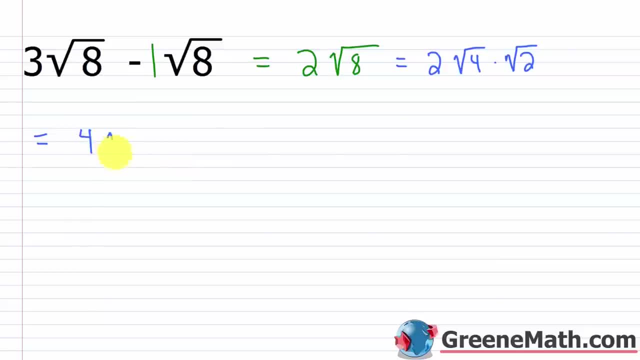 I'm going to have is what 2 times 2, or 4, times the square root of 2.. So you've got to put that extra step in there. We already know how to simplify, so once we learn how to add and. 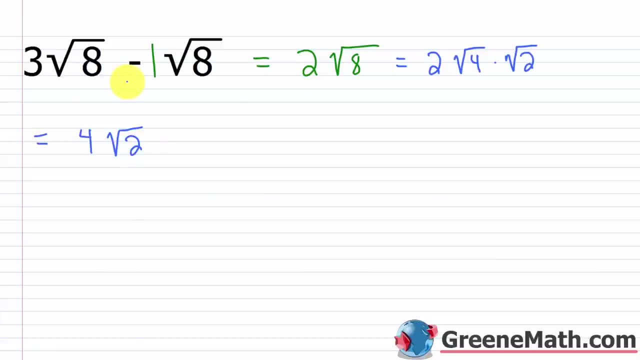 subtract. we're going to throw that extra step in of simplification that we've already learned. All right, what about something like negative 2, times the square root of 3, minus 5 times the square root of 3?? So I'm just looking at this. 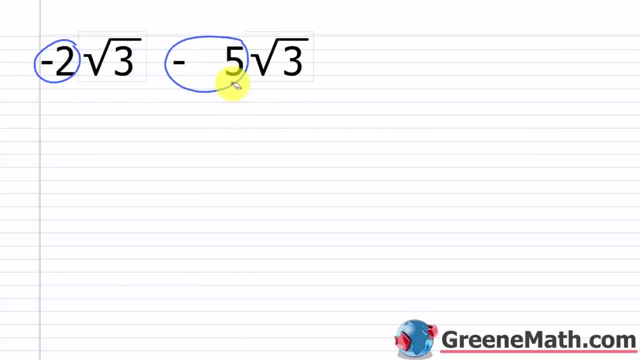 and really this right And the negative 5. there you can think about it as plus negative 5 or minus 5.. Again, whatever makes you feel more comfortable. But essentially I just think about negative 2 plus negative 5, and that's going to give me what Negative 7.. And then I have square root of 3. 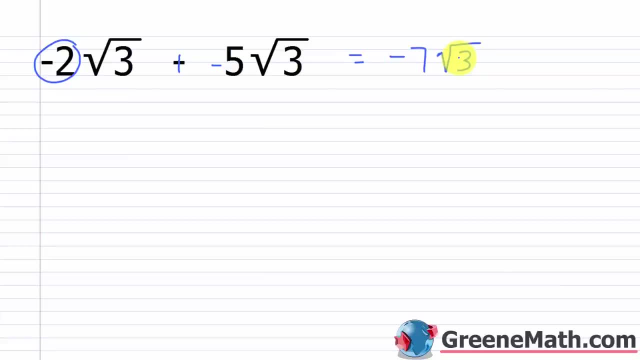 that's just coming along for the ride. So this equals negative 7 times the square root of 3, and there's nothing I can do to rewrite that. So I'm going to write negative 2 times the square root of 3,. 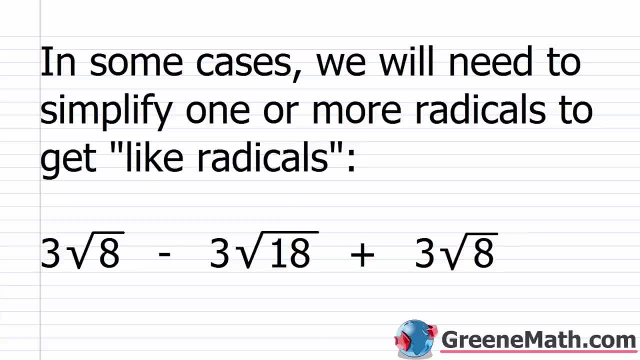 and then I'm going to write negative 2 times the square root of 3, and then I'm going to write negative 2 times the square root of 3, and then I'm going to write negative 2 times the square root of 3.. All right, so the previous examples were kind of the easy ones, the ones you get at the 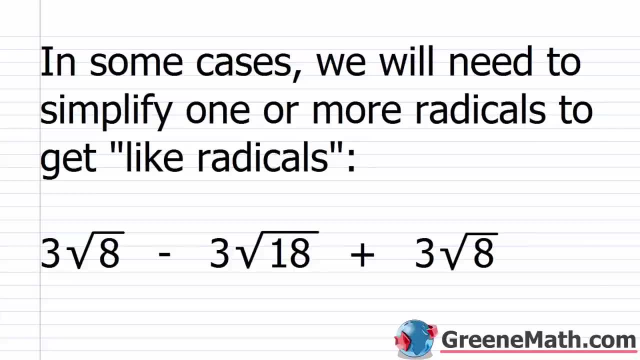 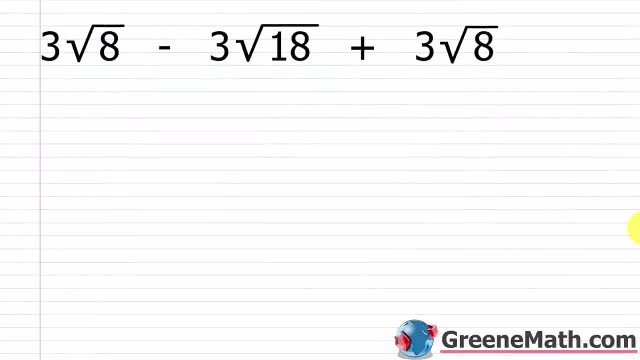 very start of this section. Then you start getting to stuff that's a little bit more complicated. So I have here that in some cases we will need to simplify one or more radicals to get like radicals. So you might get some problems that involve addition and subtraction where you look. that I can kind of work with. So I've got to leave it in that format. 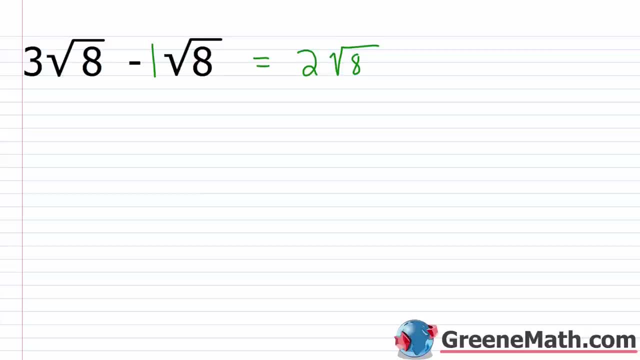 In this example, if I factored 8, I could make it 4 times 2. 4 is a perfect square, so I got to get that out of there. So let's, re-write this as 2 times square root of 4 times square root of 2. 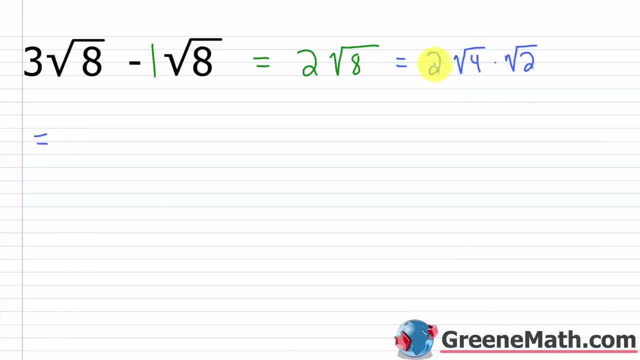 I know the square root of 4 is 2. So essentially what I'm going to have is what? 2 times 2 or 4 times the square root of 2. 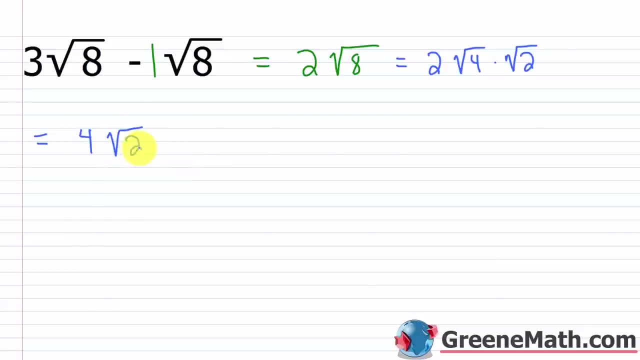 So you've got to put that extra step in there. We already know how to simplify. So once we learn how to add and subtract, we're going to throw that extra step in of simplification that we've already learned. All right. 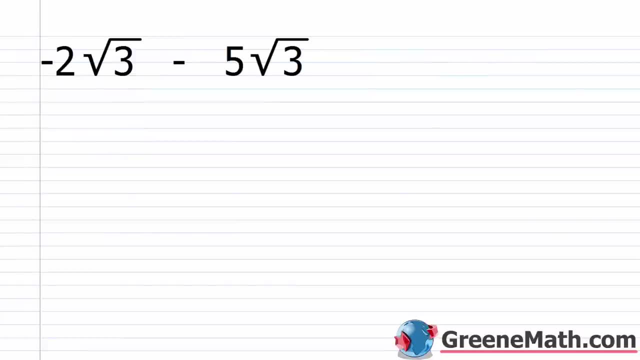 What about something like negative 2 times the square root of 3 minus 5 times the square root of 3? So I'm just looking at this and really this, right? And the negative 5 there, you can think about it as plus negative 5 or minus 5. Again, whatever makes you feel more comfortable. But essentially, 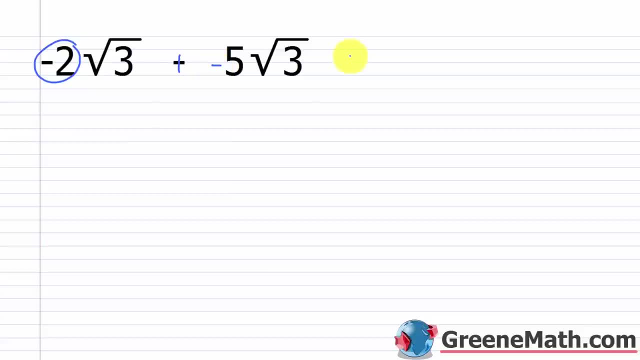 I just think about negative 2 plus negative 5. And that's going to give me what? Negative 7. 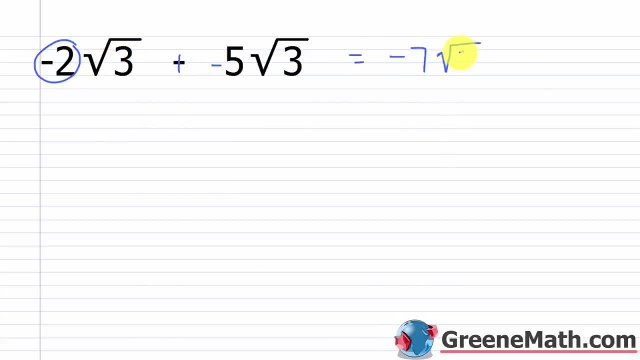 And then I have square root of 3 that's just coming along for the ride. So this equals negative 7 times the square root of 3. And there's nothing I can do to really simplify that any further. All right. 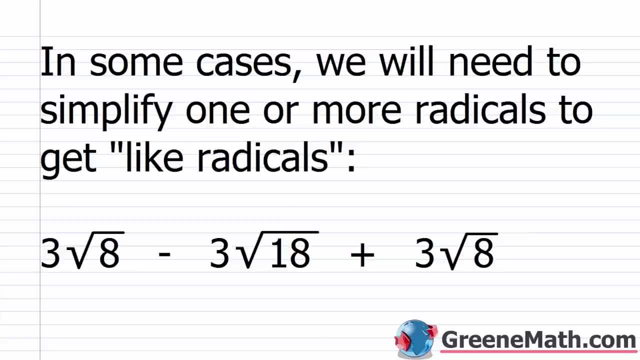 So the previous examples, we're kind of the easy ones, the ones you get at the very start of this section. 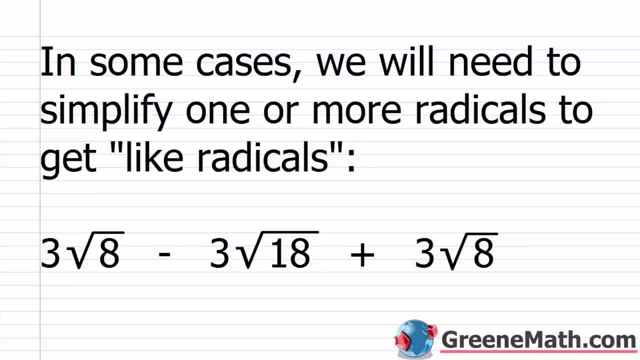 Then you start getting to stuff that's a little bit more complicated. So I have here that in some cases, 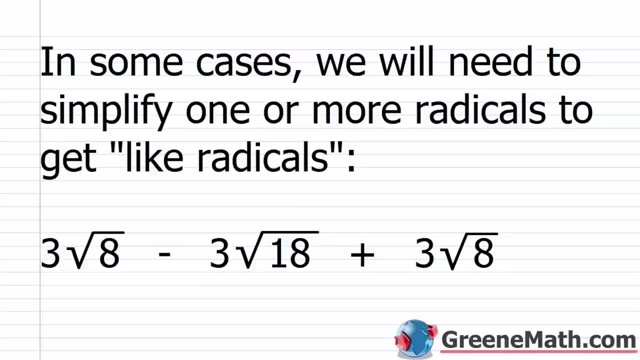 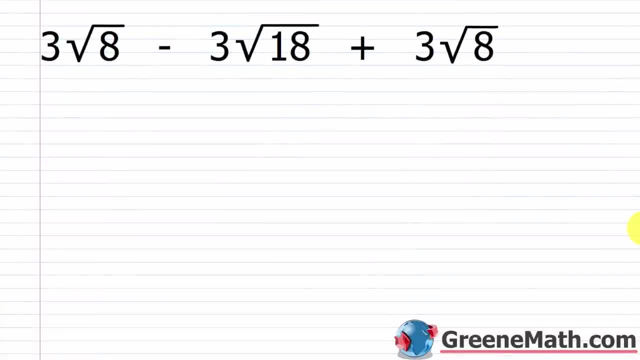 we will need to simplify one or more radicals to get like radicals. So you might get some problems that involve addition and subtraction where you look at them and it looks like you don't have like radicals, 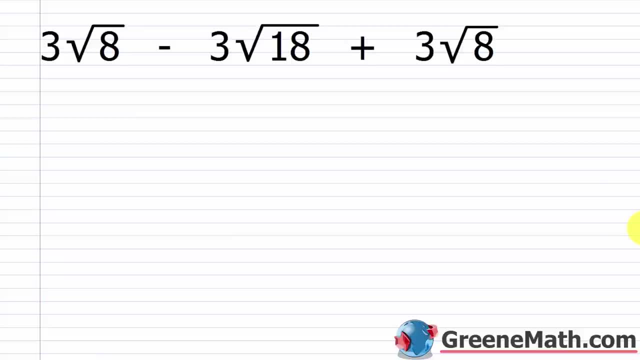 but then you do a little simplifying and it turns out that you do have like radicals. So for example, here I have 3 times the square root of 8. 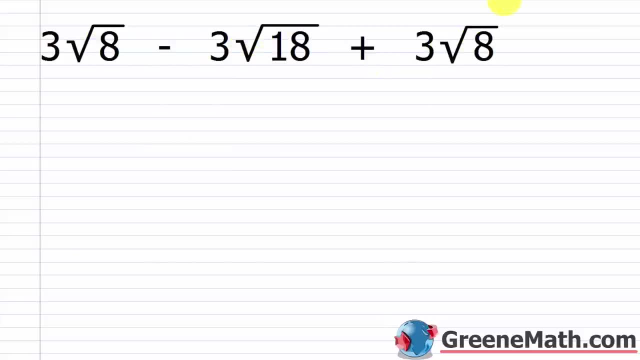 Minus 3 times the square root of 18 plus 3 times the square root of 8. So obviously these are like radicals. It's the exact same thing. So they can be added together, 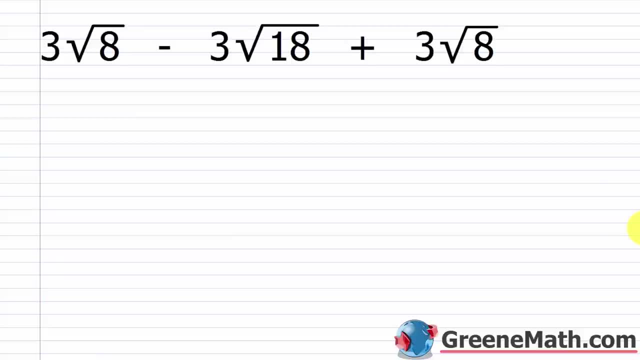 at them and it looks like you don't have like radicals. but then you do a little simplifying and it turns out that you do have like radicals. So for example, here I have 3 times the square root of 8 minus 3 times the square root of 18. 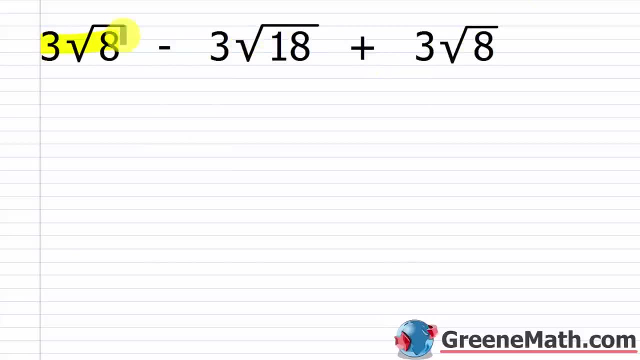 plus 3 times the square root of 8.. So obviously these are like radicals. It's the exact same thing, so they can be added together, but this is not a like radical. with anything, I have the square root of 18.. That's not going to work right, because the radicand is different. 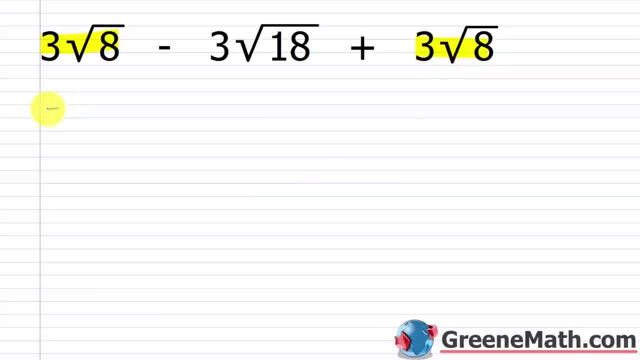 but if I go ahead and perform the operation that I can, to start, I know, 3 plus 3 is 6, so I'd have 6 times the square root of 8.. square root of 8, and then minus 3 times the square root of 18.. So what I want to do now is: 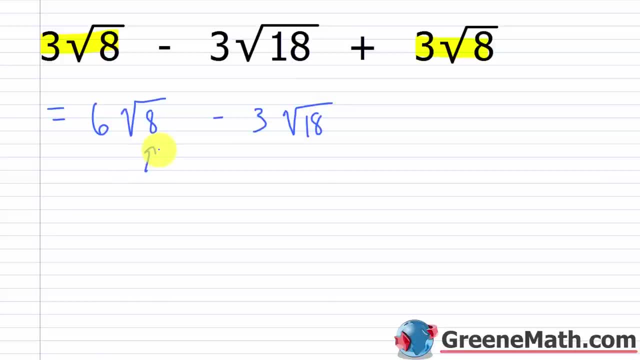 just think about simplifying each one of these. So if I think about the square root of 8, I know I could write that as the square root of 4 times the square root of 2. And this is 6 out here. 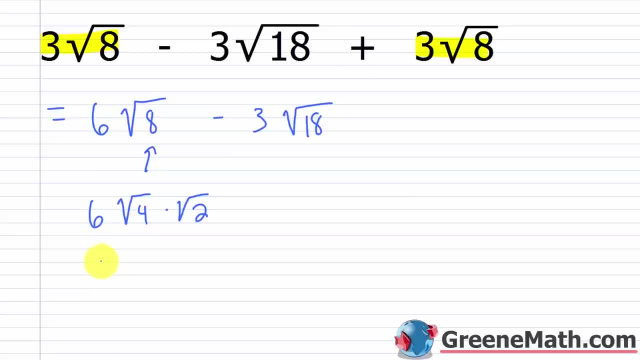 so square root of 4 is 2.. So I'd have 6 times 2 times the square root of 2, or 12 times the square root of 2.. So let's write that this equals 12 times the square root of 2.. Now for this guy. 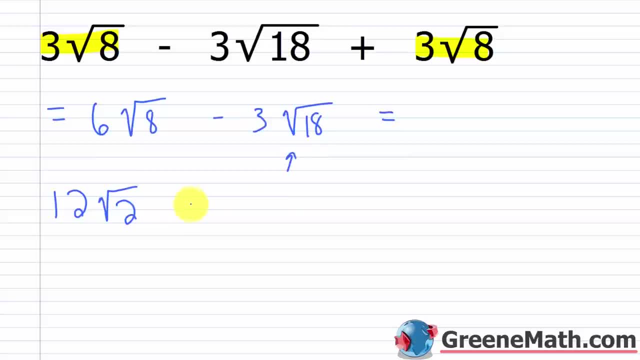 right here I've got what I've got: 3 times the square root of 18.. I could write: the square root of 9 times the square root of 2.. Now, 9 is a perfect square, so the square root of 9 is 3.. 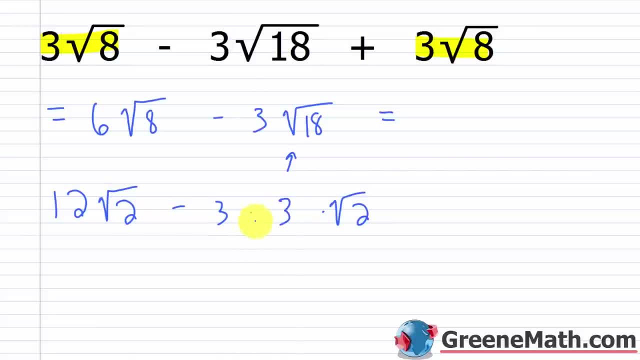 So I could write this as a 3 here: 3 times 3 is 9.. So if I replace all this, I'd really have minus 9 times the square root of 2.. And voila, we can see that we have the same radicand now: a 2 in each case and the same. 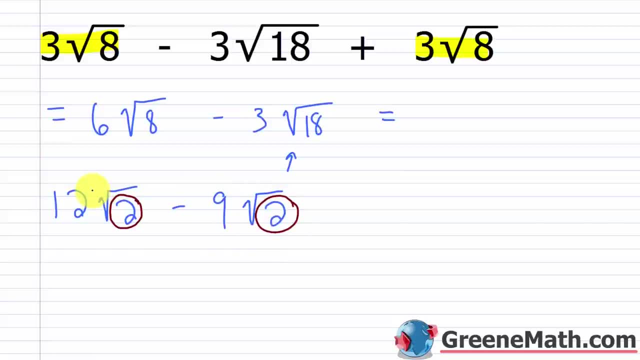 index also a 2 in each case, because this is square roots we're dealing with. So I can do this operation now. I would just do 12 minus 9, that would give me 3, and then times the square root of 2,. right, And I can't simplify that any further. so that would be my answer, All right. 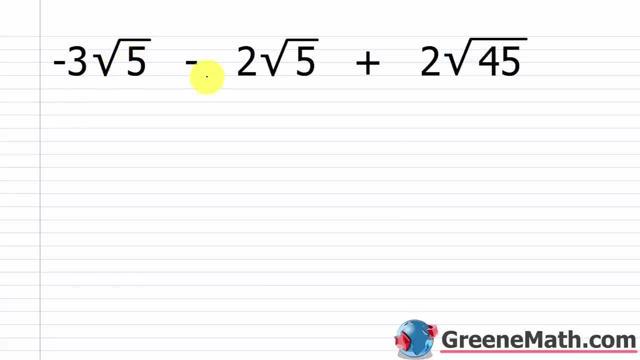 let's take a look at another one. So we have negative 3 times the square root of 5, minus 2 times the square root of 5, plus 2 times the square root of 45.. So, as we look at it, right. 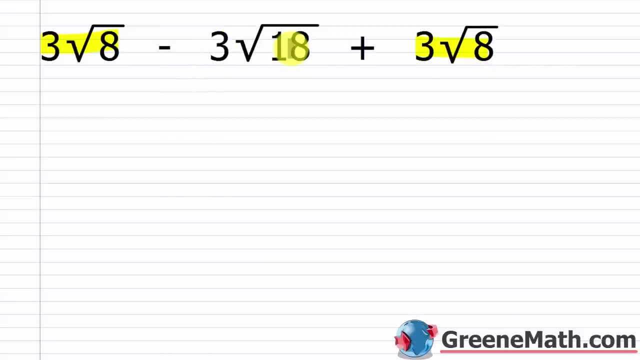 but this is not a like radical with anything. I have the square root of 18. That's, that's not going to work, right? Because the radicand is different. 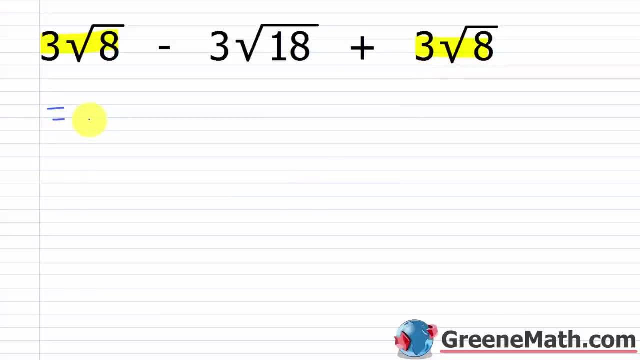 But if I go ahead and perform the operation that I can to start, I know 3 plus 3 is 6. So I'd have 6 times the square root of 8. So 6 times square root of 8. And then, minus 3 times the square root of 18. 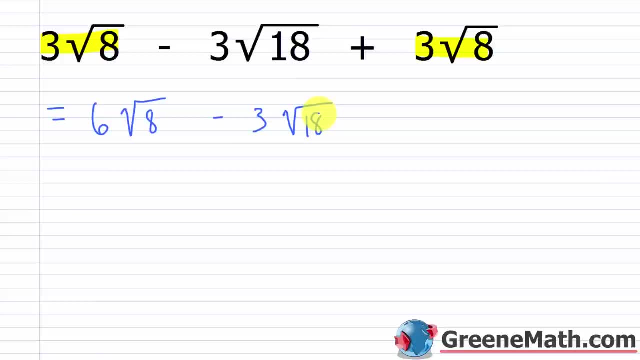 So what I want to do now is just think about simplifying each one of these. So if I think about the square root of 8, I know I could write that as the square root of 4 times the square root of 2. And this is 6 out here. So square root of 4 is 2. 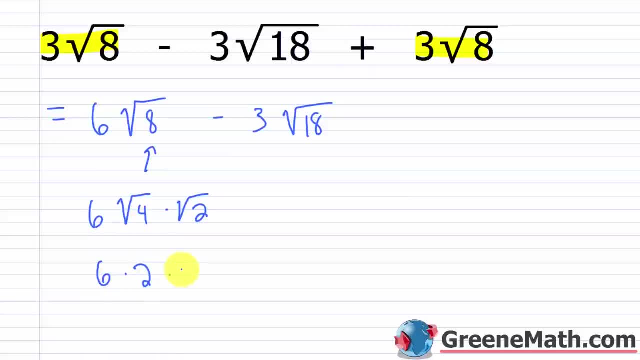 So I'd have 6 times 2 times the square root of 2 or 12 times the square root of 2. So let's write that this equals 12 times the square root of 2. Now for this guy right here I've got what. I've got 3 times square root of 18 I can write the square root of 9 times the square root of 2. Now 9 is a perfect square, so the square root of 9 is 3. 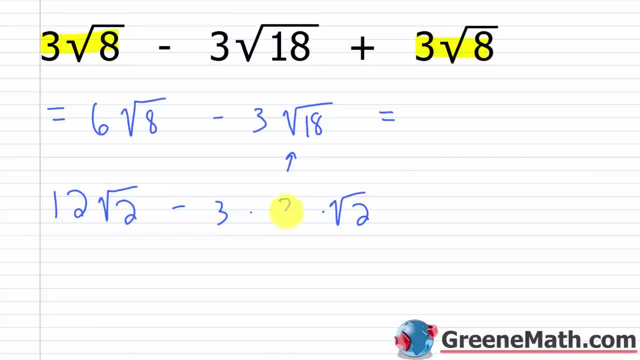 So I could write this as a 3 here. 3 times 3 is 9. 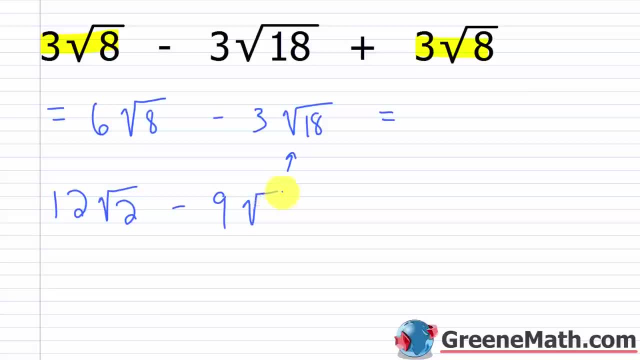 So if I replace all this, I'd really have minus 9 times the square root of 2. And voila. We can see that we have the same radicand. 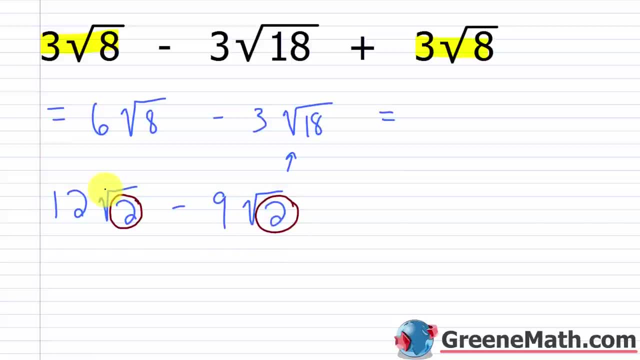 can now, a 2 in each case, and the same index, also a 2 in each case, because this is square 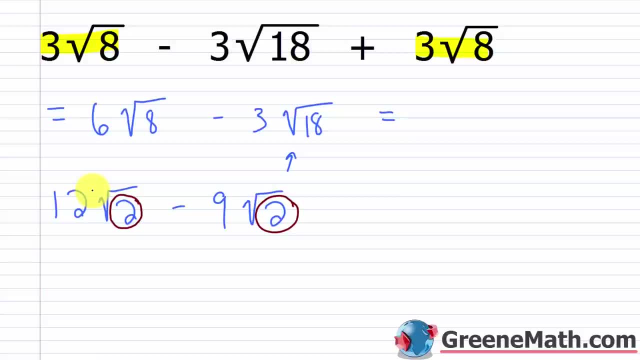 roots we're dealing with. So I can do this operation now. I would just do 12 minus 9, that would give me 3, and then times the square root of 2, right? And I can't simplify that any 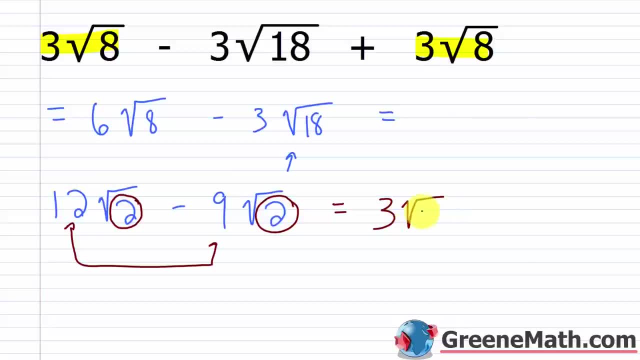 further, so that would be my answer. All right, let's take a look at another one. So we have 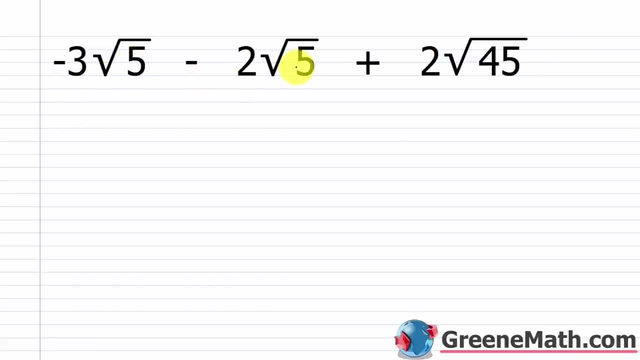 negative 3 times the square root of 5, minus 2 times the square root of 5, plus 2 times the square root of 45. So as we look at it right now, we don't have like radicals all the way across, 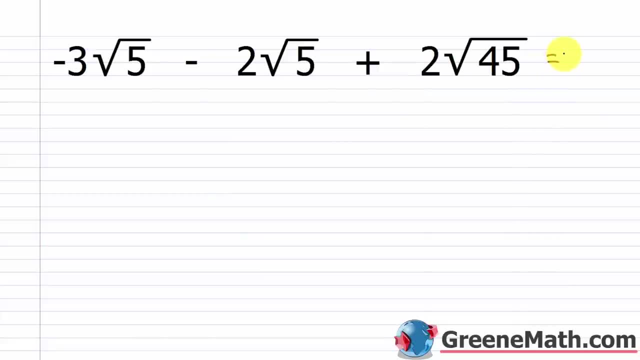 but I can perform operations with these two radicals. I can do negative 3 minus 2, that's negative 5, times the square root of 5, and then I have plus 2 times the square root of 45. 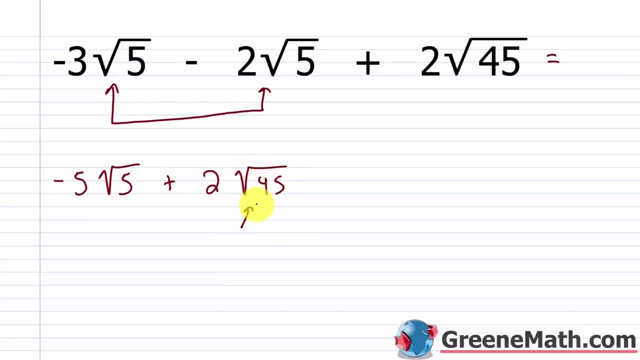 Now, I can simplify this guy, and let's see what we get. I know the square root of 45 can be written as the square root of 45 times the square root of 45, and then I can simplify this guy, so let's write that. So negative 5 times the square root of 5, plus 2 times the square root of 9, times the square root of 5. We know the square root of 9 is 3, so let's write this as negative 5 times the square root of 5, plus 2 times, again, square root of 9 is 3, times the square root of 5. So what we're going to find is that we do have like radicals. We're plus two times three is six. So this is six times square root of five. And now I can just do negative five plus six. That's going to be one. So this would end up being one times the square root of five. Or you could really just write the square root of five, right? One times anything is just 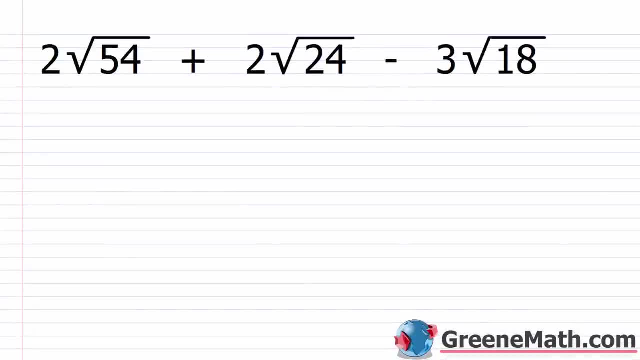 itself. All right, let's take a look at another one. So we have two times the square root of 54 plus two times the square root of 24 minus three times the square root of 18. Now, in this particular case, we don't have any like radicals to start. So I want to break down everything completely and see what I got. So I know the square root of 54. If I think about 54, I know it's nine times six. So let me do two times the square root of nine times the square root of six. 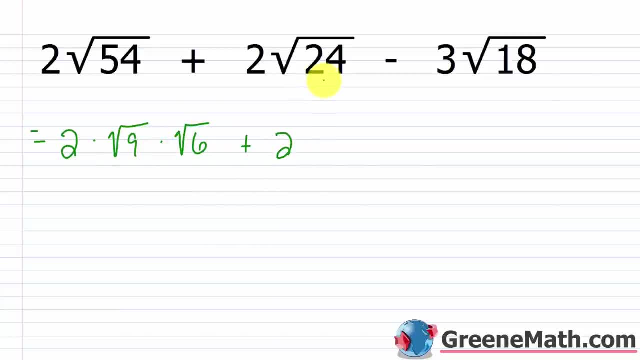 And then plus, I've got two times square root of 24. I know 24 is four times six. So let me do square root of four times square root of six. And then minus, I have three. 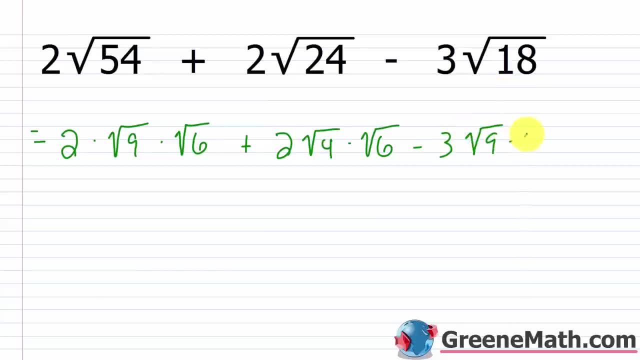 times square root of 18. So I can do square root of 9 times square root of 2. Okay, so put equals here. Square root of 9 is 3. So 2 times 3 would be 6. So this would be 6 times the square root of 6. 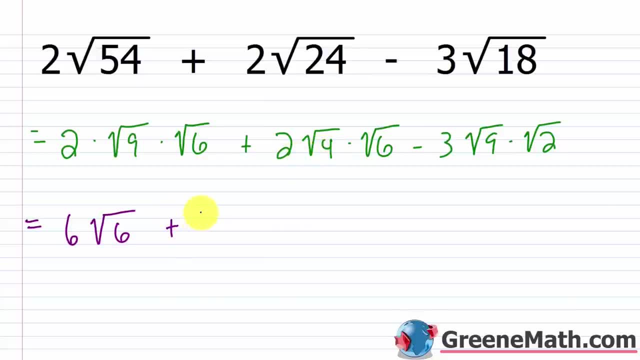 And then plus square root of 4 is 2. So 2 times 2 is 4. So 4 times square root of 6. And then minus, we have 3 here. Square root of 9 is 3. So 3 times 3 would be 9. So this would be 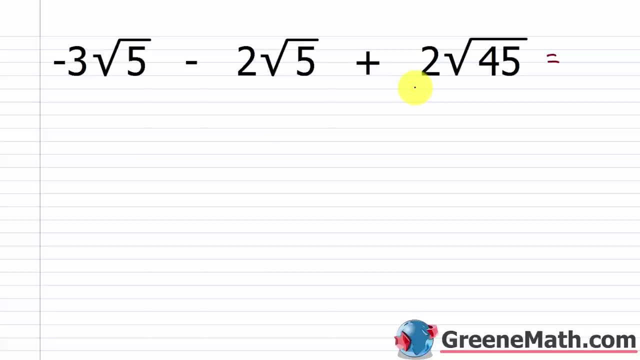 now we don't have like radicals all the way across, but I can perform operations with these two radicals. I can do negative 3 minus 2, that's negative 5, times the square root of 5, and then I have plus 2 times the square root of 45. Now I can simplify this guy and let's see what we get. 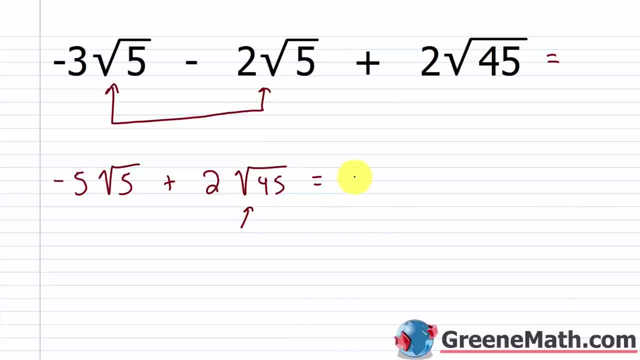 I know the square root of 45 can be written as the square root of 9 times the square root of 5.. So let's write that So negative 5 times the square root of 5, plus 2 times the square root of 9 times. 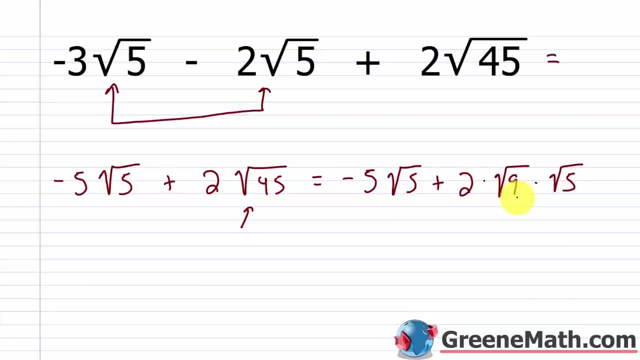 the square root of 5.. And we know the square root of 9 is 3.. So let's write this as negative: 5 times the square root of 5, plus 2 times again: square root of 9 is 3, times the square root of 5.. So 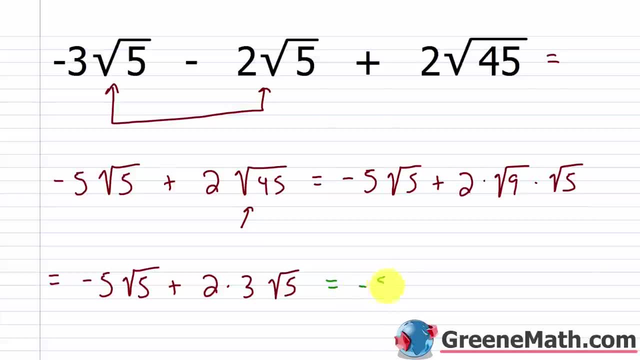 what we're going to find is that we do have like radicals. We're going to have negative 5 times the square root of 5 plus 2 times 3 is 6, so this is 6 times square root of 5, and now I can just do negative. 5 plus 6, that's going to be 1, so this would end up being 1 times. 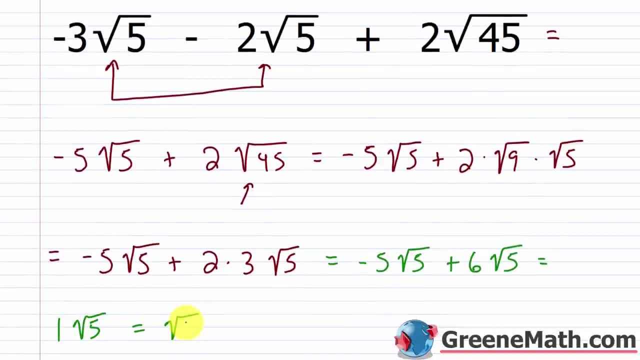 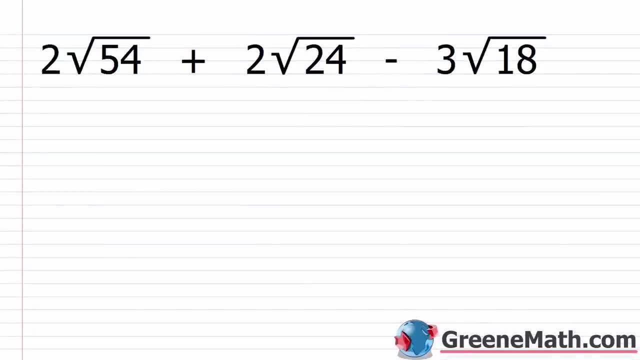 the square root of 5, or you could really just write the square root of 5, right, 1 times. anything is just itself. all right, let's take a look at another one. so we have 2 times the square root of 54 plus 2 times the square root of 24, minus 3 times the square root of 18. now, in this particular, 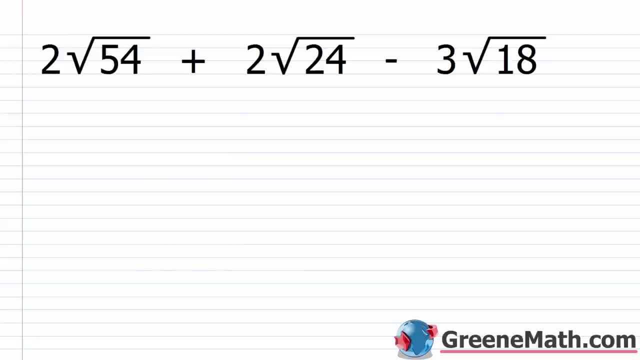 case. we don't have any like radicals to start, so I want to break down everything completely and see what I got. so I know the square root of 54. if I think about 54, I know it's 9 times 6, so let me do. 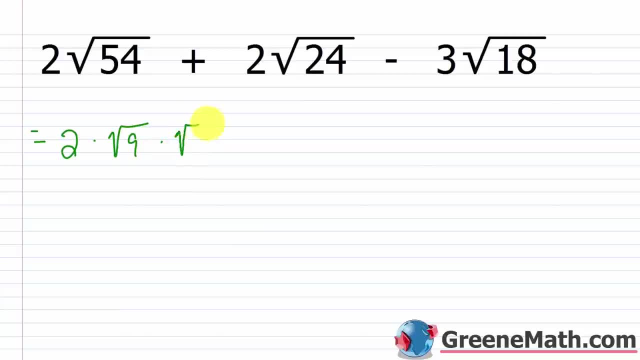 2 times the square root of 9, times the square root of 6, and then plus, I've got 2 times square root of 24. I know 24 is 4 times 6, so let me do square root of 4 times square root of 6 and then. 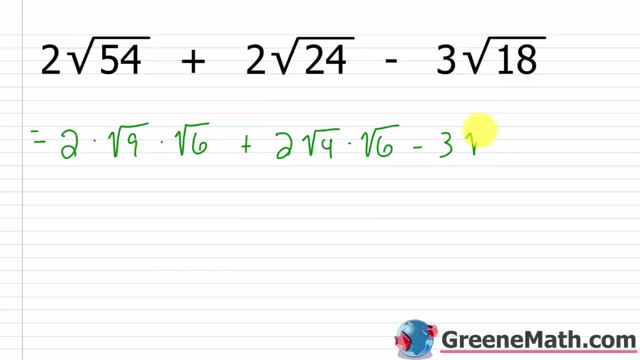 minus, I have 3 times the square root of 18, so I can do square root of 9 times square root of 2. okay, so put equals here. square root of 9 is 3, so 2 times 3 would be 6, so this would be 6 times the square root of 6. 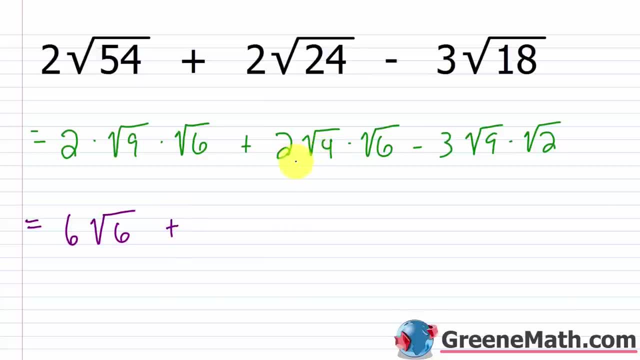 and then plus square root of 4 is 2, so 2 times 2 is 4, so 4 times square root of 6, and then minus we have 3. here square root of 9 is 3, so 3 times 3 would be 9. so this would be. 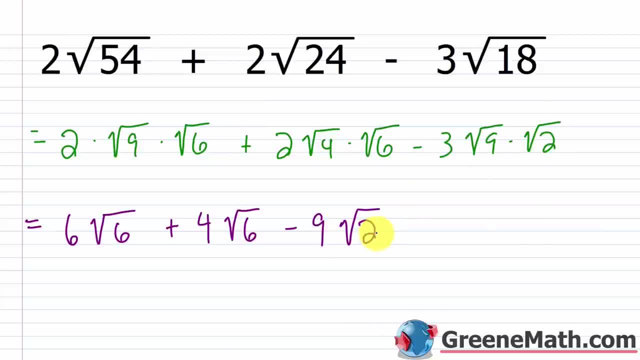 minus 9 and then times the square root of 2. now I have like radicals for these two. This one is not. I have square root of 2 here. I have square root of 6 here and here, So you've got to have like radicals to combine these okay. 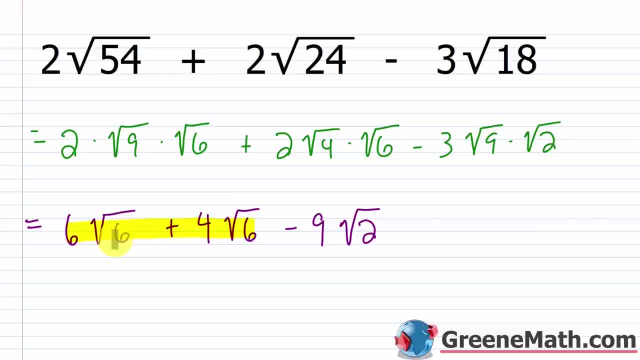 You can't just combine them if they're not like radicals. I see that mistake all the time. Don't do that. So what we're going to do is just combine what we can. So in other words, I would say: 6 plus 4 is 10, so this would be 10 times the square root. 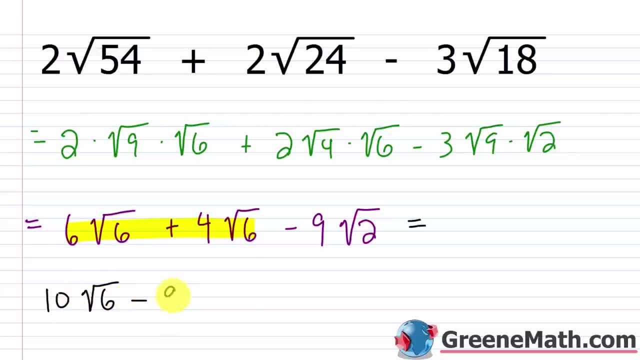 of 6, can't make that any simpler- then minus 9 times the square root of 2.. This is all that I can do. I can do no more here. okay, Now, this is kind of similar to if you had something like, let's say, you simplified as. 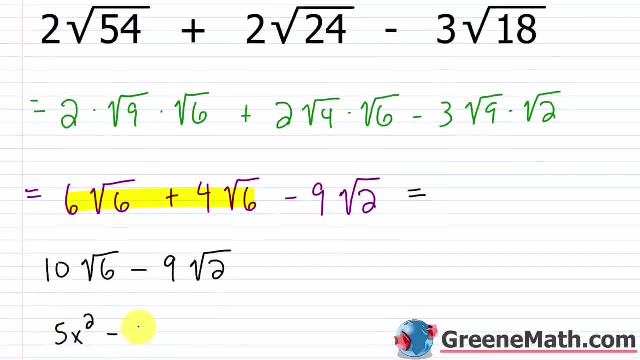 much as you could and you had 5x squared minus 3x. let's say These aren't like terms, so I can't go any further. That's my simplified answer. It's the same thing here. They're not like radicals in this case, so I can't simplify any further. 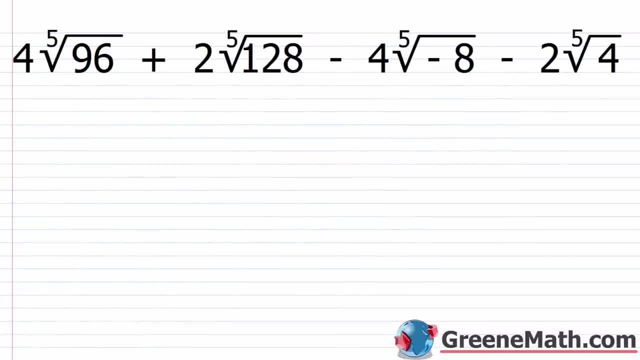 So let's take a look at one more. and if you understood the main lesson on radicals and you understood how to simplify, I think that this particular topic, within the topic of radicals, is pretty simple overall. So if I look at 4 times the 5th root of 96 plus 2 times the 5th root of 128 minus 4 times, 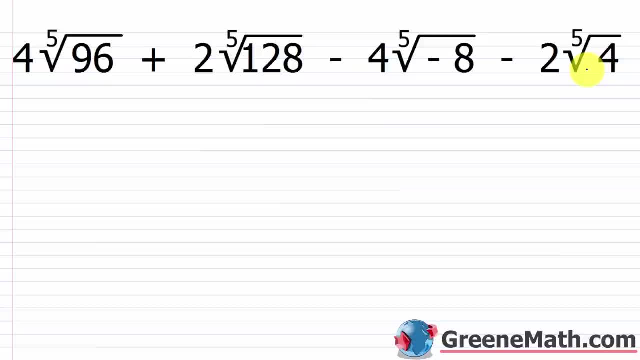 the 5th root of negative 8 and then minus 2 times the 5th root of 4, I don't have any like radicals to start, so I've got to look and see what I can do, So let's start with just 96.. 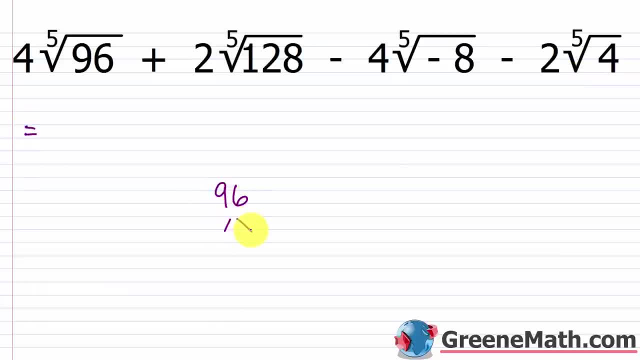 If I think about 96, I know that would factor in a 32 times 3.. Now 32 is 2 to the 5th power, so I already can see that I can do what: 4 times the 5th root of 32, times the 5th root of 3.. 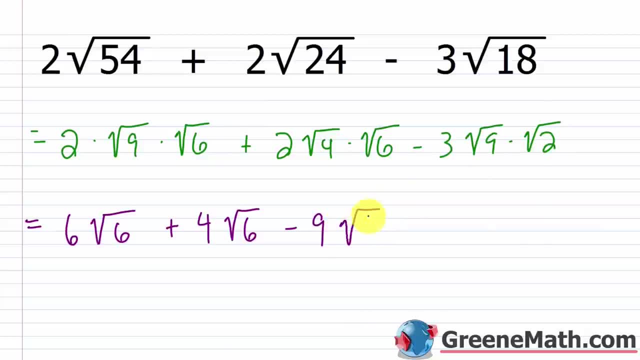 4 minus 9 and then times the square root of 2. Now, I have like radicals for these two. This one is not. I have square root of 2 here. I have square root of 6 here and here. So you've got to have like radicals to combine these. Okay, you can't just combine them if they're not like 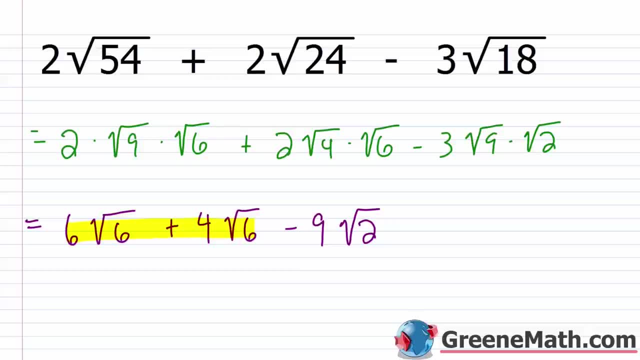 radicals. I see that mistake all the time. Don't do that. So what we're going to do is just combine what we can. So in other words, I would say 6 plus 4 is 10. So this would be 10. 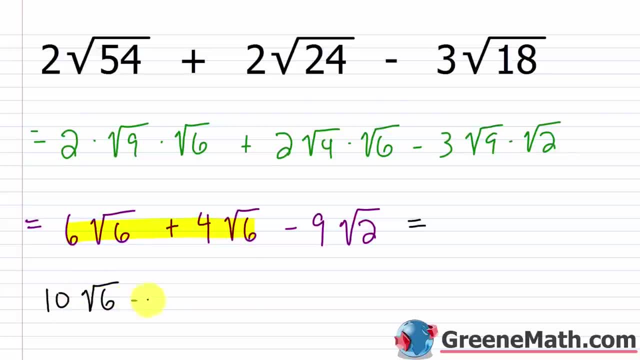 Times the square root of 6. Can't make that any simpler. Then minus 9 times the square root of 2. This is all that I can do. I can do no more here. Okay. Now, this is kind of similar to if you had 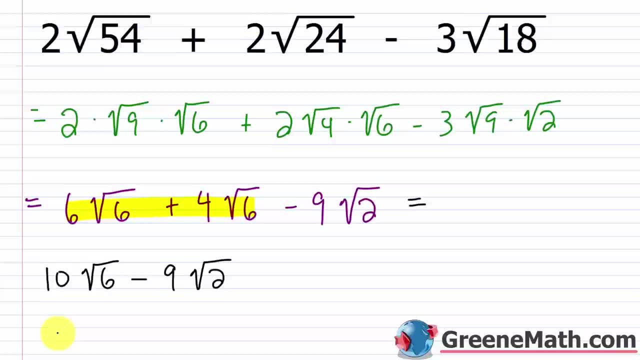 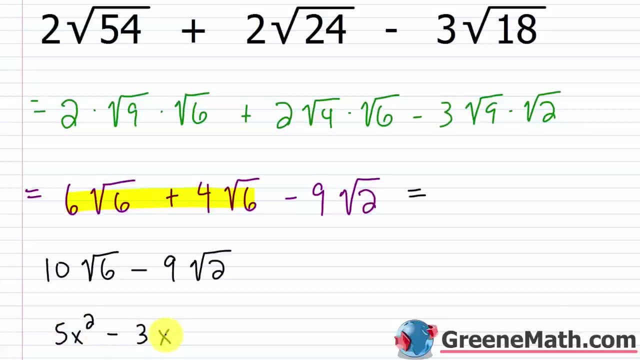 something like, let's say you simplified as much as you could and you had 5x squared minus 3x, let's say. These aren't like terms. So I can't go any further. That's my simplified answer. 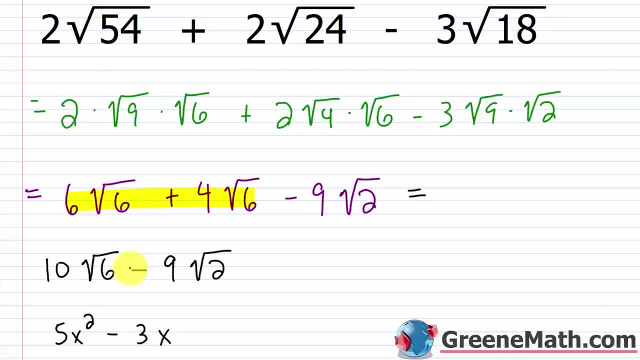 It's the same thing here. They're not like radicals in this case. So I can't simplify. 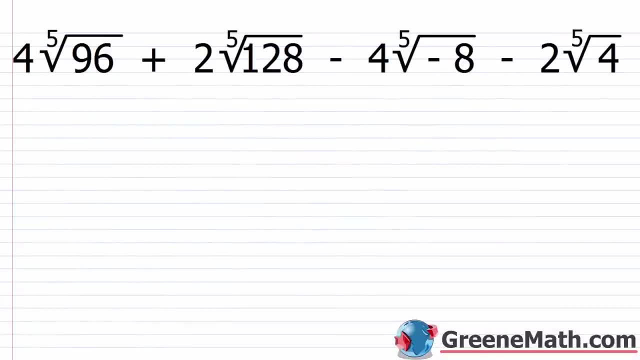 So let's take a look at one more. And if you understood the main lesson on radicals and you understood how to simplify, I think that this particular topic within the topic of radicals is pretty simple overall. So if I look at 4 times the 5th root of 96 plus 2 times the 5th root of 128 minus 4 times the 5th root of negative 8 and then minus 2 times the 5th root of 4, 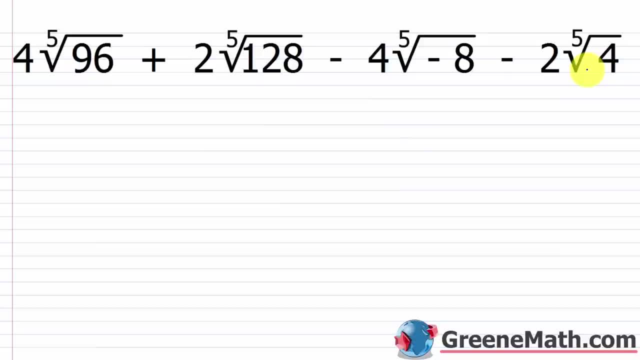 I don't have any like radicals to start. So I've got to look and see what I can do. 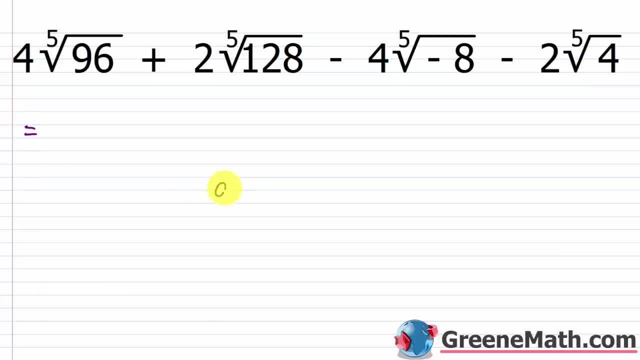 So let's start with just 96. If I think about 96, I know that would factor in a 32 times 3. Now, 32 is 2 to the 5th power. So I already can see that I can do what? 4 times the 5th root of 32 times the 5th root of 3. And just to kind of save myself a little time, I can just kind of simplify this as I go. Again, 2 to the 5th power. So I can do 4 times the 5th root of 32 times the power is 32. So I know the 5th root of 32 is 2. So I can put that this is going to be 2. And of course, if I multiply 4 times 2, I get 8. So let's just, again, save ourselves a little bit of time and put 8 times the 5th root of 3. Okay, so let's try to simplify this one now. I think at this point that we all know that 128 is 2 to the 7th power. So if I have 2 to the 7th power and I have something that's an index of 5. Again, you got to kind of think about these things to speed yourself up. I would think about this as 2 to the 5th power times 2 squared. 2 to the 5th power is 32. So I'm going to break this up and say I have 2 times the 5th root of 32 times the 5th root. 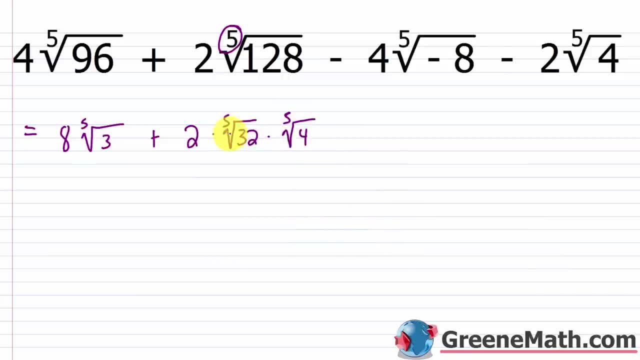 2 squared would be what? That's 4. So I already know that the 5th root of 32 is 2. 2 times 2 is 4. So this is going to be 4 times. 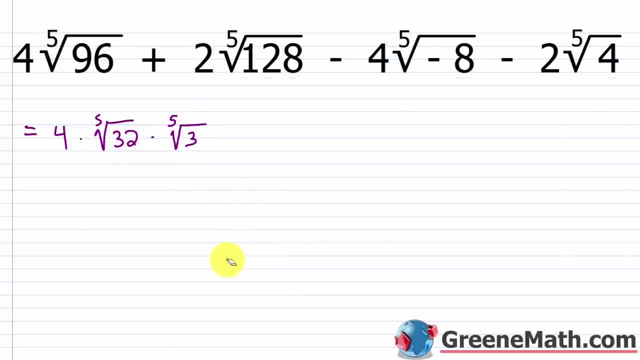 And just to kind of save myself a little time, I can just kind of simplify this as I go Again: 2 to the 5th power minus 4 times the 5th root of 3.. Okay, The 5th power is 32, so I know the 5th root of 32 is 2.. 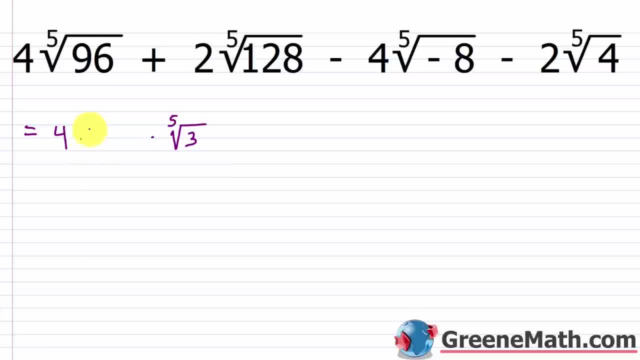 So I can put that this is going to be 2 and of course, if I multiply 4 times 2,, I get 8.. So let's just again save ourselves a little bit of time and put 8 times the 5th root of. 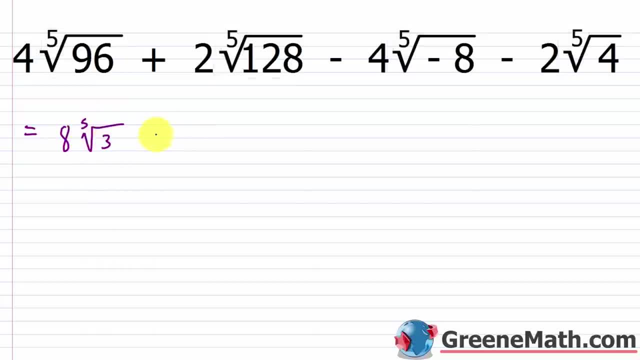 3. Okay, so let's try to simplify this one now. I think at this point that we all know that 128 is 2 to the 7th power. So if I have 2 to the 7th power And I have something that's an index of 5.. 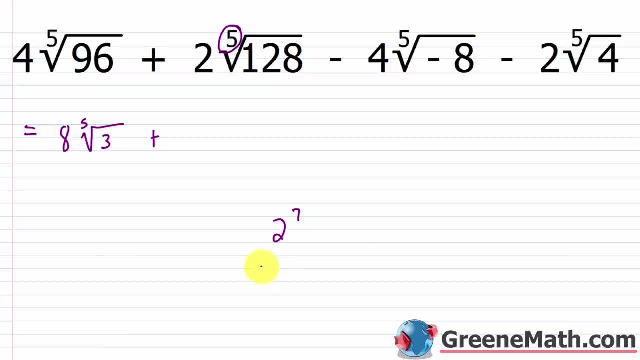 Again, you got to kind of think about these things. to speed yourself up, I would think about this as 2 to the 5th power, times 2, squared 2 to the 5th power is 32.. So I'm going to break this up and say I have 2 times the 5th root of 32 times the 5th root. 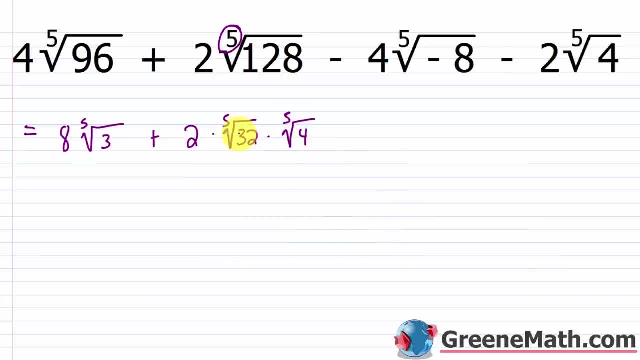 2 squared would be what That's 4.. So I already know that the 5th root of 32 is 2.. 2 times 2 is 4.. So this is going to be 4 times Okay. So this is going to be 4 times the 5th root of 4.. 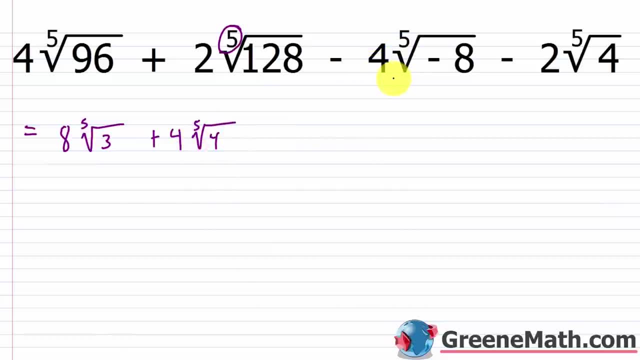 So now I want to think about negative 4 times the 5th root of negative 8.. Is there anything I can do to simplify there? Well, it looks like I can't, but actually I can do a little trick with that. 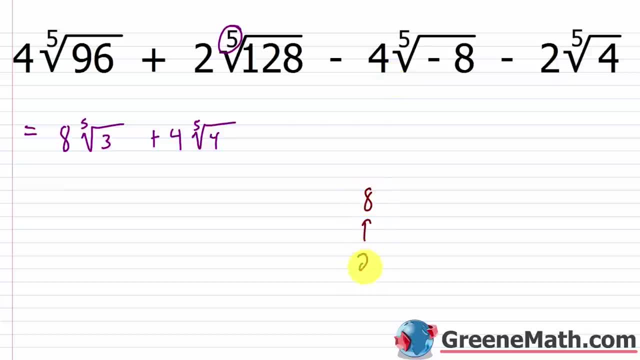 Now, if you think about 8, it's what It's: 2 cubed Now 3 isn't high enough to match up with this index of 5 to be able to simplify it that way. But I can do something with the negative right. 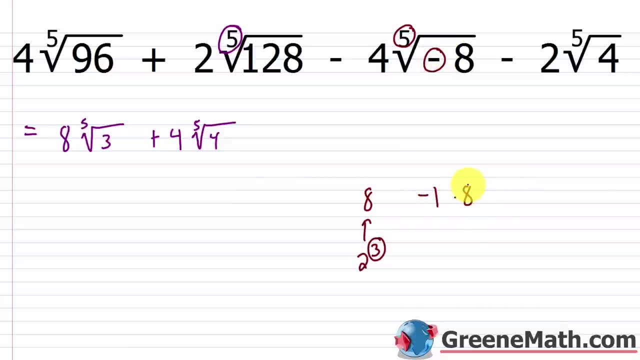 If you think about that as what Negative 1 times 8, okay, and then the negative 1 raised to the 5th power would give me negative 1.. So I can think about it as saying that I can actually pull out a negative 1 from this. 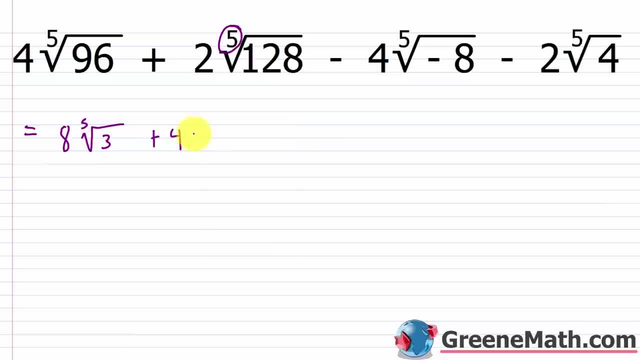 4 times the 5th root of 4. So now I want to think about negative 4 times the 5th root of negative 8. Is there anything I can do to simplify there? Well, it looks like I can't, but actually I can do a little trick with that. Now, if you think about 8, it's what? It's 2 cubed. Now, 3 isn't high enough to match up with this index of 5 to be able to simplify in that way. I can't do anything with the 8. But I can do something. With the negative, right? If you think about that as what? Negative 1 times 8. Okay. And then the negative 1 raised to the 5th power would give me negative 1. So I can think about it as saying that I can actually pull out a negative 1 from this. And let me show you how you go about doing that. So let's write plus negative 4. And then times, I'm going to put the 5th root of negative 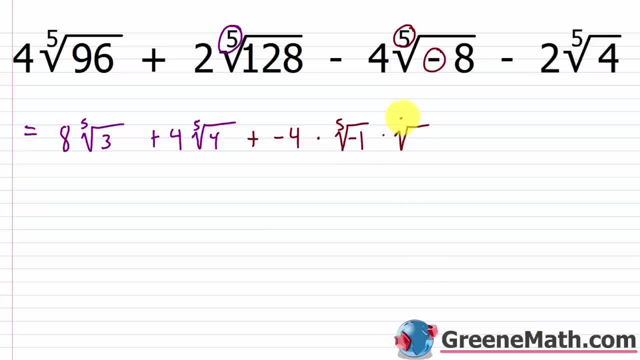 1. And then times the 5th root. 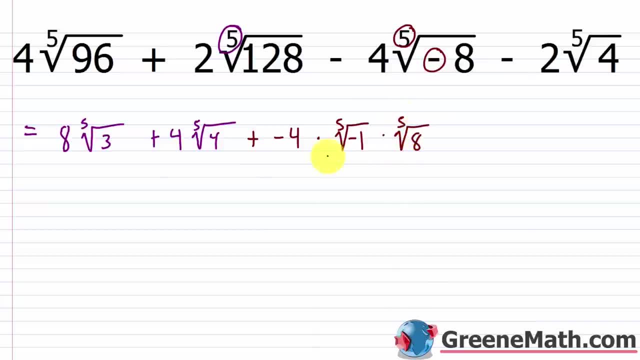 Of 8. Okay. And again, I'm legally allowed to do that per the product rule for radicals. Haven't done anything illegal. Now, what is the 5th root of negative 1? It's negative 1, right? If I took negative 1 and I multiplied by itself 5 times, I'd get negative 1. So I can erase this and just put negative 1 here. Now, I can simplify now by saying negative 4 times negative 1 is positive 4. So this would be positive 4 times negative 1. And then I can write minus 2 times the 5th root of positive 8 now. Okay. So not a simplification in the normal way that you'd expect, but a way to kind of clean it up a little bit. Then we have minus 2 times the 5th root of 4. And nothing I can do with that, right? If I think about 4, it's just 2 times 2. Can't really do anything with that. So I only have like radicals here and here. So all I'm going to be able to do in this scenario is combine those. So I'm going to be able to combine those. 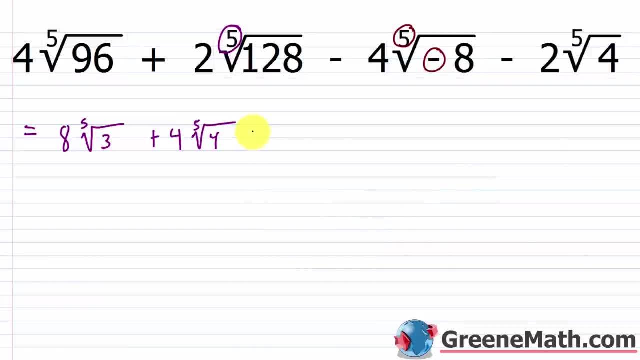 And let me show you how you go about doing that. So let's write: plus negative 4 and then times- I'm going to put the 5th root of negative 1.. And then times the 5th root of 8, okay. 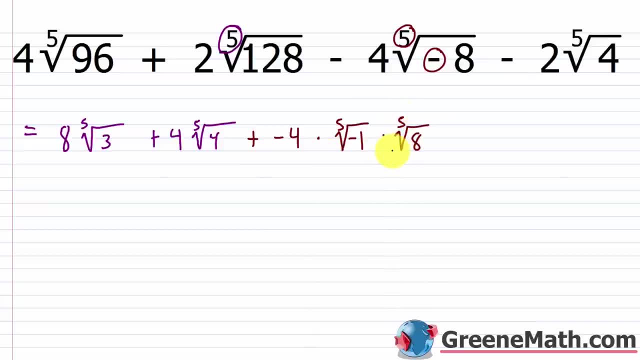 And again, I'm legally allowed to do that per the product rule for radicals. I haven't done anything illegal. Now what is the 5th root of negative 1? It's negative 1, right? If I took negative 1 and I multiplied by itself 5 times, I'd get negative 1.. 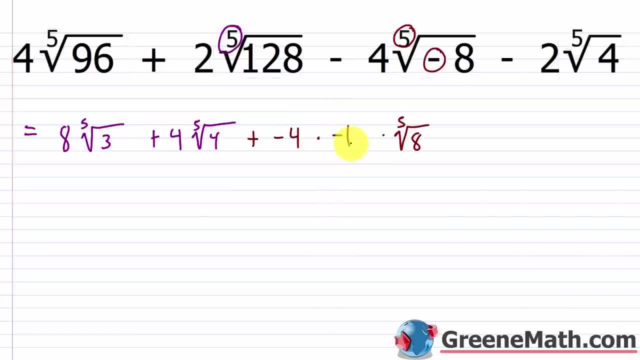 So I can erase this and just put negative 1 here Now. I can simplify now by saying: negative 4 times negative 1 is positive 4.. So this would be positive 4 times the 5th root of positive 8. now okay, 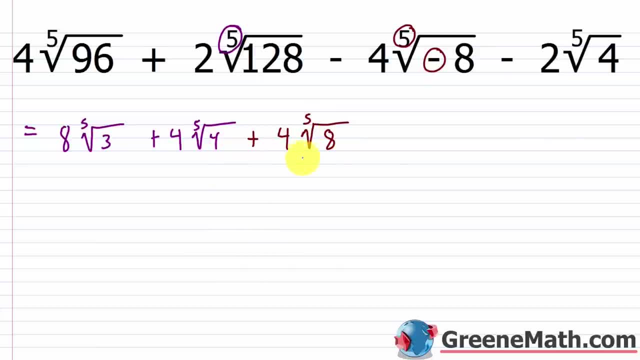 So not a simplification in the normal way that you'd expect, but a way to kind of clean it up a little bit. Then we have minus 2 times the 5th root of 4. And nothing I can do with that, right. 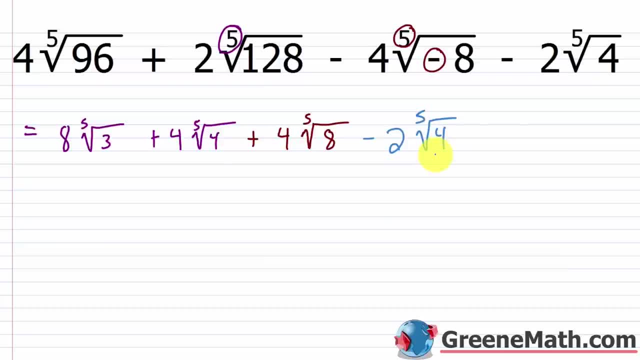 If I think about 4, it's just 2 times 2, can't really do anything with that, So I only have like radicals here and here. So all I'm going to be able to do in this scenario is combine those. 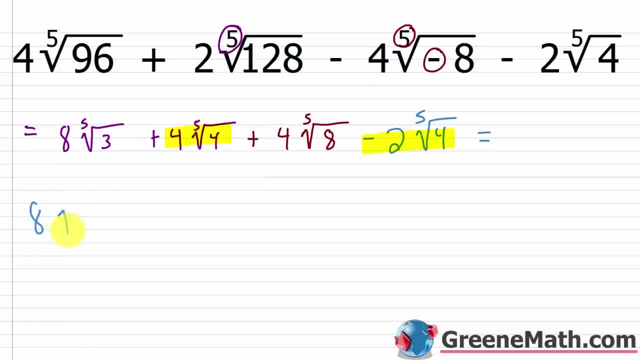 So if I look at this, I'm going to have what? 8 times the 5th root of 3.. And then plus I can do 4 minus 2, that's 2 times the 5th root of 4.. 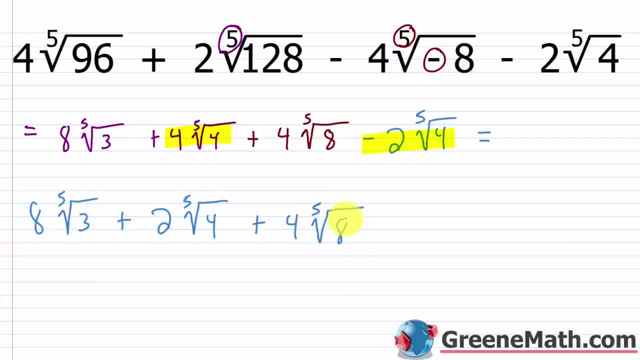 And then plus 4 times the 5th root of 8.. And again, these are not like radicals, so there's nothing else I can do to combine or simplify any further. Hello And welcome to Algebra 1, Lesson 2.. 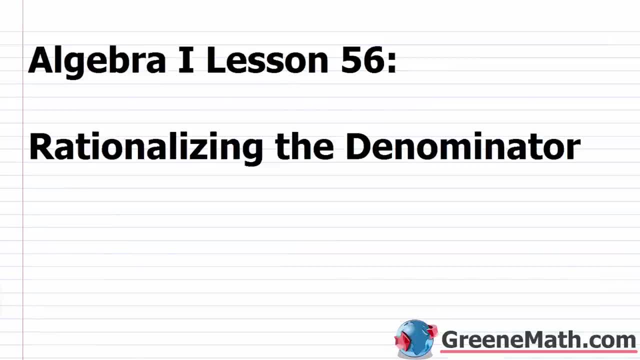 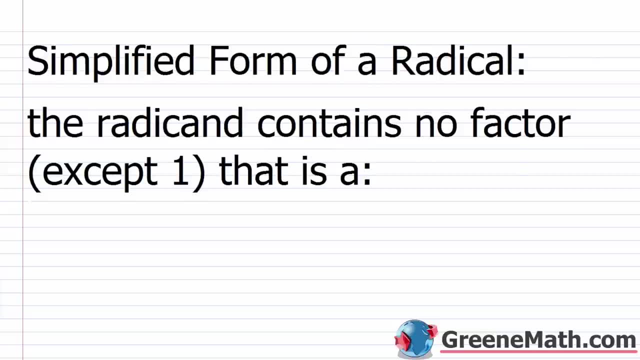 Okay, So we're going to look at what a simplified radical is. In this video we're going to learn about rationalizing the denominator. All right, So before we kind of move on in Algebra 1, we need to learn what a simplified radical 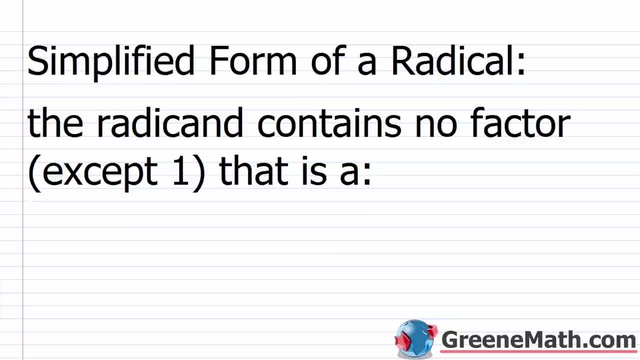 is Just like when we work with fractions. we always had to simplify it before we reported our answer. we're going to be expected to do the same thing when we work with radicals. So there's three main things you have to do when you work with radicals. 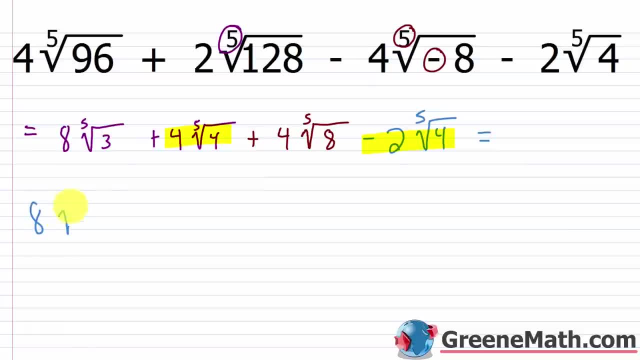 So I'm going to be able to combine those. So I'm going to be able to combine those. So I'm going to If I look at this, I'm going to have what? 8 times the 5th root of 3. And then plus, I can do 4 minus 2. That's 2 times the 5th root of 4. And then plus 4 times the 5th root of 8. And again, these are not like radicals. So there's nothing else I can do to combine or simplify any further. 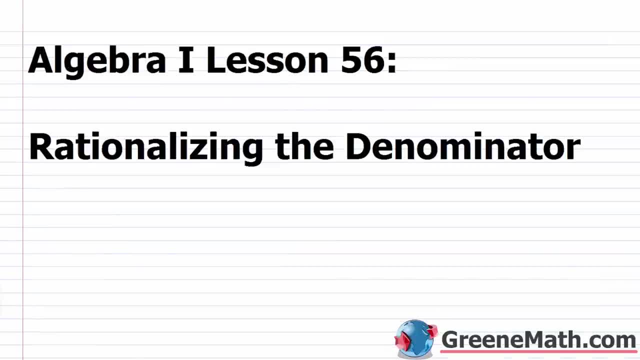 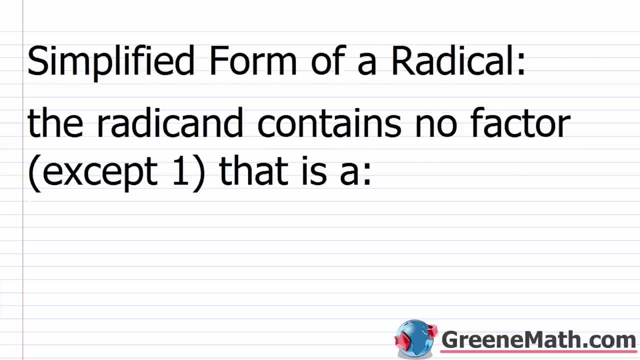 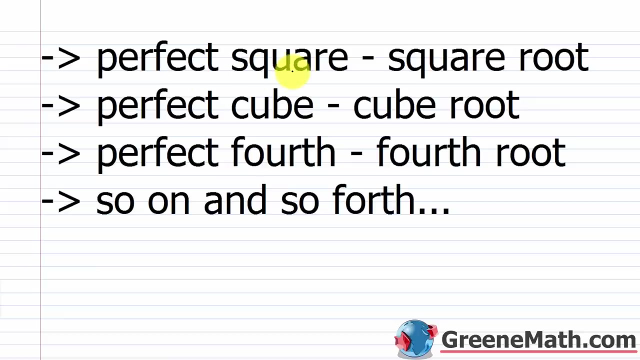 Hello and welcome to Algebra 1 Lesson 56. In this video, we're going to learn about rationalizing the denominator. All right, so before we kind of move on in Algebra 1, we need to learn what a simplified radical is. Just like when we work with fractions, we always had to simplify it before we reported our answer. We're going to be expected to do the same thing when we work with radicals. So there's three main things you have to do when you work with radicals. So I have here that the simplified form of a radical, and this is kind of the first thing. The radicand, remember that's your number or your radical. So the radical is the number of your variable or could be your expression that's under your radical sign. This contains no factor except for one, that is a. We have perfect square in the case of a square root, perfect cube in the case of a cube root, perfect fourth in the case of a fourth root, and then so on and so forth. So what we're basically saying is that if you saw something like the square root of 8, 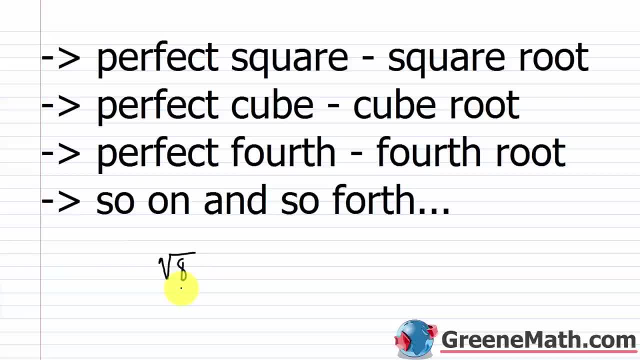 8 has a factor of 4, right? 4 is a perfect square. So because this is a square root, this is not simplified because one of the factors of 8 is a perfect square. I could write this as the square root of 4 times the square root of 2, and then the square root of 4 is 2. So I can write this as 2 times the square root of 2. So we've been doing this for a few lessons now, so we already understand this concept. But this goes for higher powers as well. If I had something like, let's say the cube root of 16, I know that 8 is a factor of 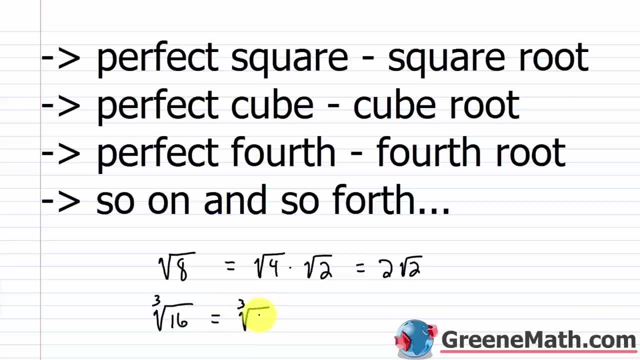 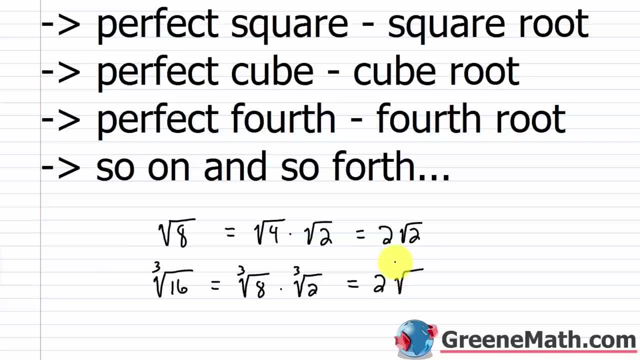 4. So I could write this as the cube root of 8 times the cube root of 2, and then the cube root of 8 is 2. So this is 2 times the cube root of 2. So that's one of the things you're looking for 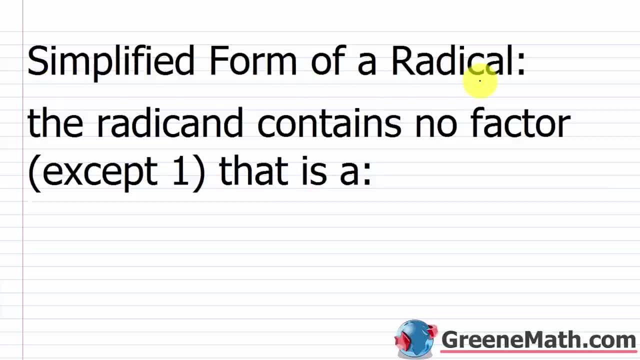 So I have here that, the simplified form of a radical, and this is kind of the first thing, the radicand, remember that's your number or your variable, or could be your expression, that's under your radical sign. This contains no factor, except for 1, that is a. 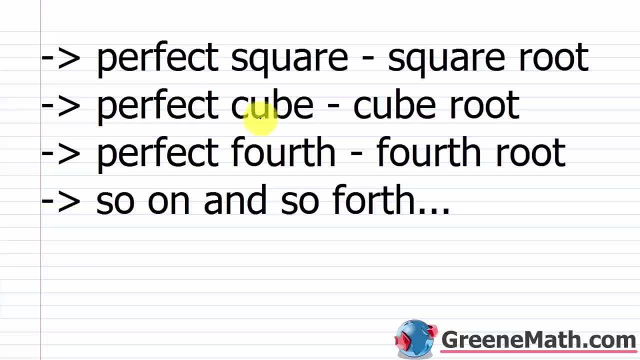 We have perfect square in the case of a square root. perfect cube in the case of a cube root. perfect fourth in the case of a fourth root, and then so on and so forth. So what we're basically saying is that if you saw something like the square root of 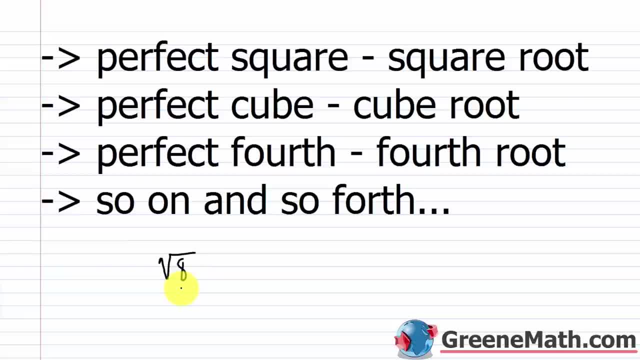 8.. 8 has a factor. 8 has a factor. 8 is a square root of 4.. 4 is a perfect square. So, because this is a square root, this is not simplified, because one of the factors of 8 is a perfect square. 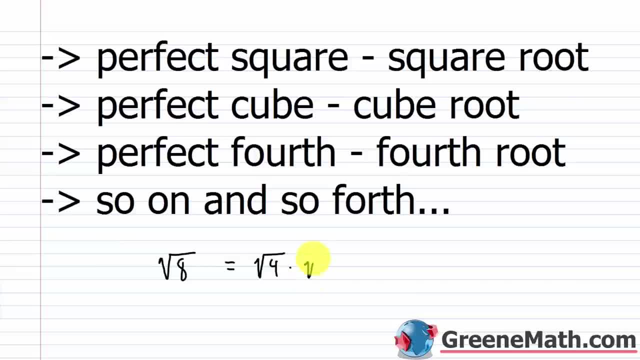 I can write this as the square root of 4 times the square root of 2, and then the square root of 4 is 2, so I can write this as 2 times the square root of 2.. So we've been doing this for a few lessons now, so we already understand this concept. 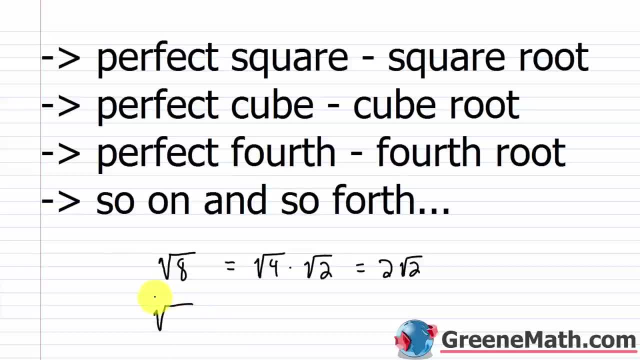 But this goes for higher powers as well. If I had something like, let's say, the cube root of 16.. I know that 8 is a factor of 16 and 8 is a perfect cube, So I could write this as the cube root of 8 times the cube root of 2.. 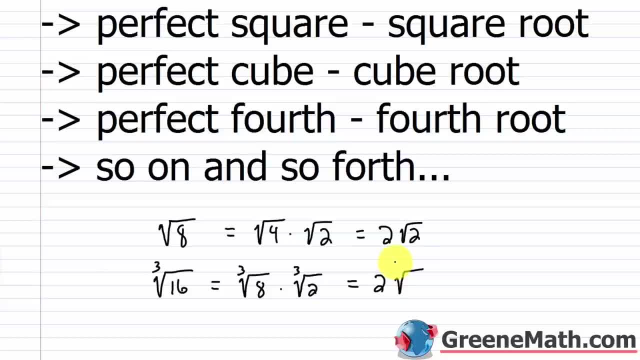 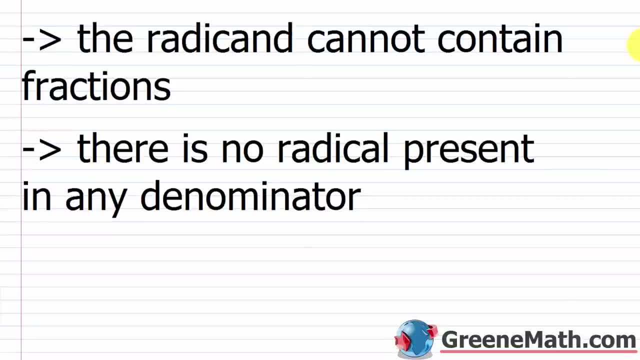 And then the cube root of 8 is 2.. So this is 2 times the cube root of 2.. So that's one of the things you're looking for when you're simplifying a radical. All right. the next thing, and we've already learned how to kind of deal with this scenario. 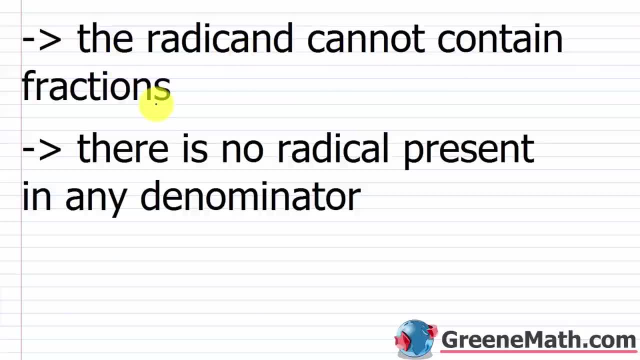 The radicand cannot contain fractions. Okay, So if you have something like, let's say, the square root of 1- 4th, you've got to split that up and say that this is equal to the square root of 1 over the square root of 4.. 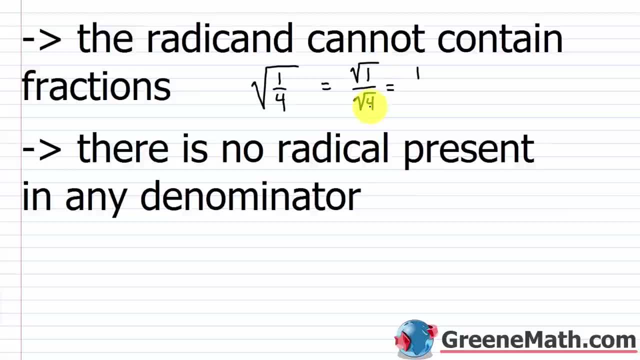 And of course this is something you could simplify: Square root of 1 is 1.. Square root of 4 is 2.. So that becomes 1: half. But you can't leave it in this format. The radicand: again, this is the number or the variable or the expression that is underneath the radical symbol. 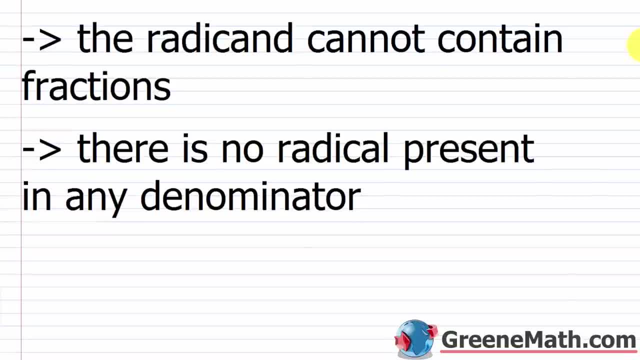 when you're simplifying a radical. All right, the next thing, and we've already learned how to kind of deal with this scenario, the radicand cannot contain fractions, okay? So if you have something like, let's say the square root of 1.5, you can write this as the square root of 1.5. So if you have something like, let's say the square root of 1.5, you can write this as the square root of 1.5. So you've got to split that up and say that this is equal to the square root of 1 over the square root of 4. And of course, this is something you could simplify. Square root of 1 is 1, square root of 4 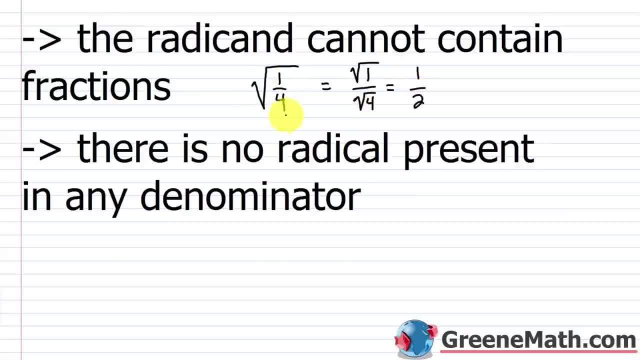 is 2, so that becomes 1.5. But you can't leave it in this format. The radicand, again, this is the 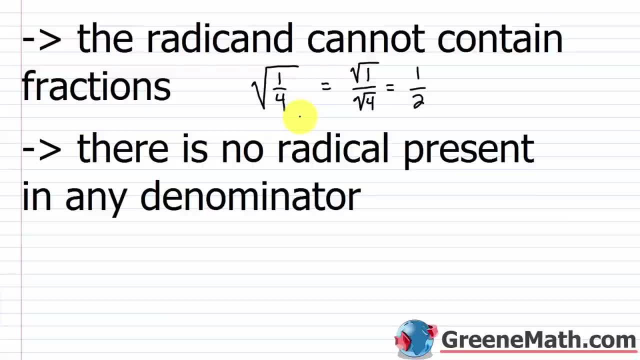 number or the variable or the expression that is underneath the radical symbol, cannot contain fractions when you report your simplified answer. 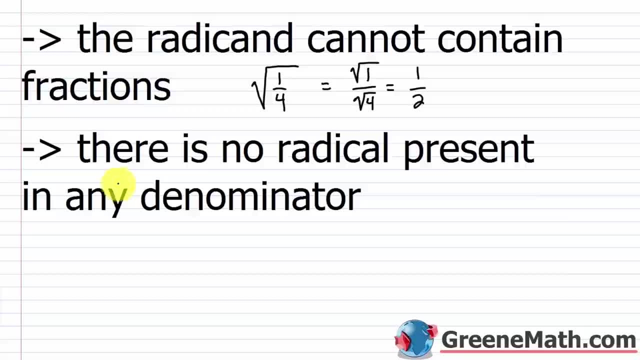 Then there's the last thing here, that is, there is no radical present in any denominator. So we can't have something like, let's say 2 over the square root of 5, or something like 6 over the square root of 7. They don't want that. That's considered not simplified. So basically, the purpose of this lesson is to teach you how to deal with these scenarios right here. We've already learned how to simplify this, and then also how to deal with these scenarios right here. So if you want to learn how to simplify this, you can also start with the first thing we talked about, which 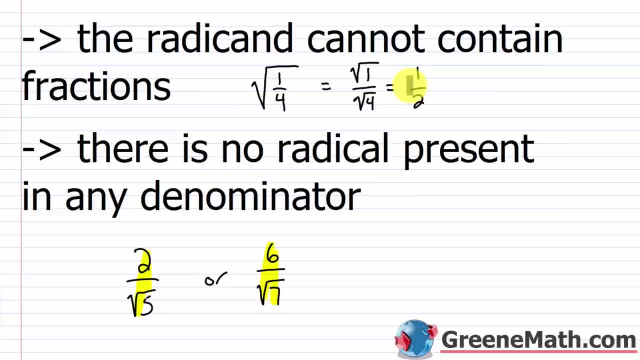 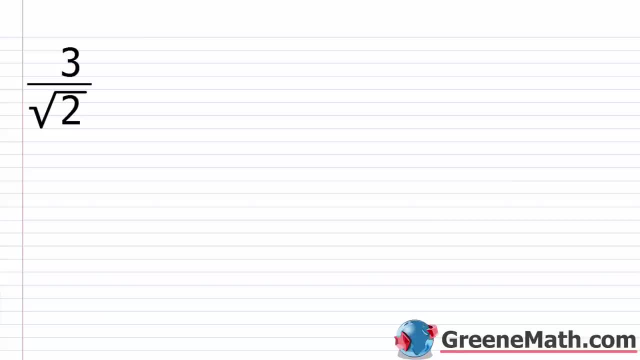 is pulling out a perfect square, or pulling out a perfect cube. So we're focusing on this in this lesson. So what do I do when I come across something like 3 over the square root of 2? Again, we cannot have a radical in the denominator. So this right now is called an irrational number. 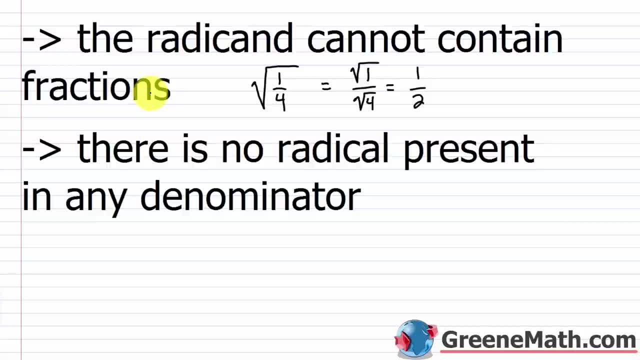 cannot contain fractions when you report your simplified answer. Then there's the last thing here, That is, there is no radical present in any denominator, So we can't have something like, let's say, 2 over the square root of 5.. 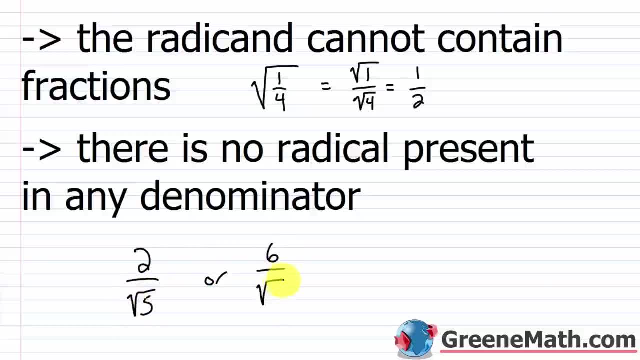 Or something like 6 over the square root of 7.. They don't want that. That's considered not simplified. So basically, the purpose of this lesson is to teach you how to deal with these scenarios. right here, We've already learned how to simplify this. 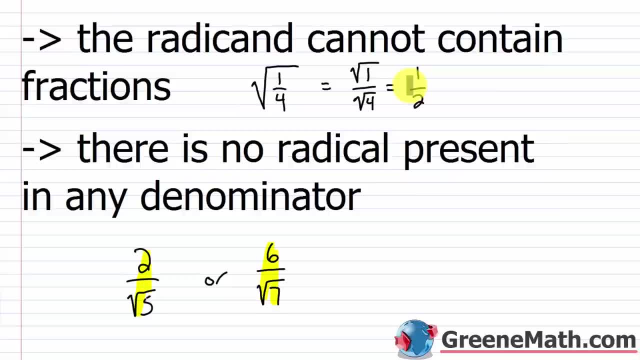 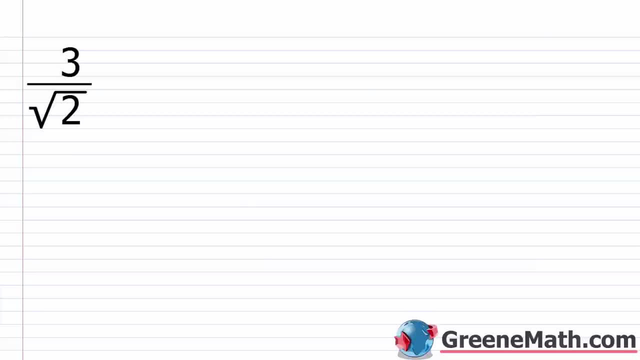 And then also kind of the first thing we talked about, which is, you know, pulling out a perfect square or pulling out a perfect cube. So we're focusing on this in this lesson. So what do I do when I come across something like 3 over the square root of 2?? 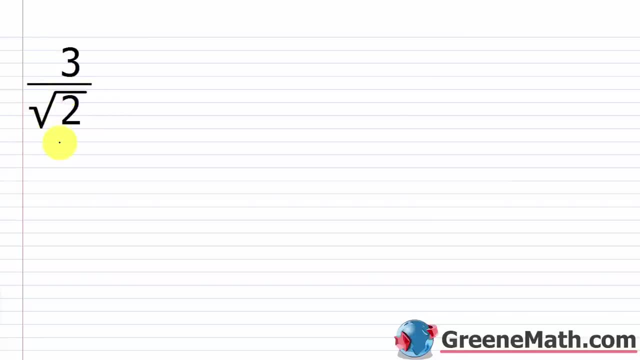 Again, we cannot have a radical in the denominator, So this right now is called an irrational number. This is an irrational number. We don't want this, So what could we possibly do to get rid of it? Well, I didn't say that I couldn't have a radical in the numerator. 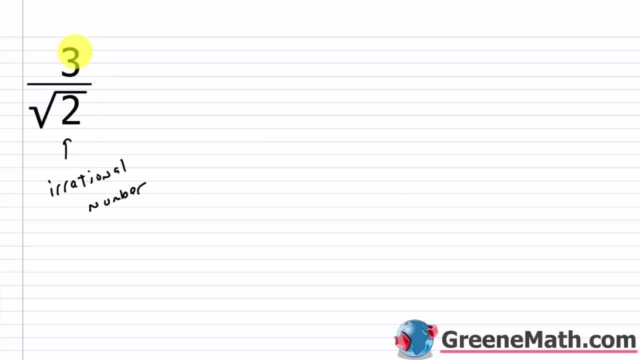 If I just don't want one in the denominator, all I need to do is perform a little trick that we learned back when we studied fractions: I'm going to multiply the denominator by the square root of 2. And I'm going to do the same thing to the numerator. 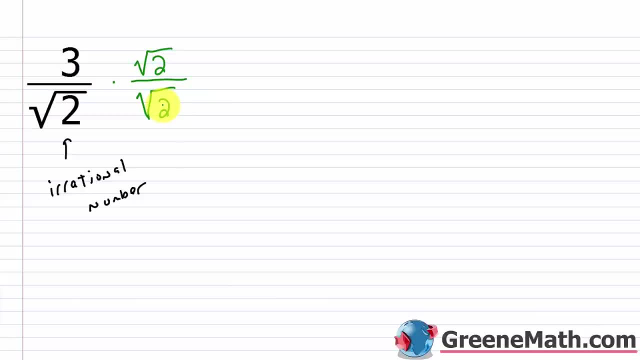 Remember, the square root of 2 over the square root of 2 is a complicated form of 1.. Same non-zero number over itself: It's 1.. Okay, Now what happens when I multiply the square root of 2 times the square root of 2?? 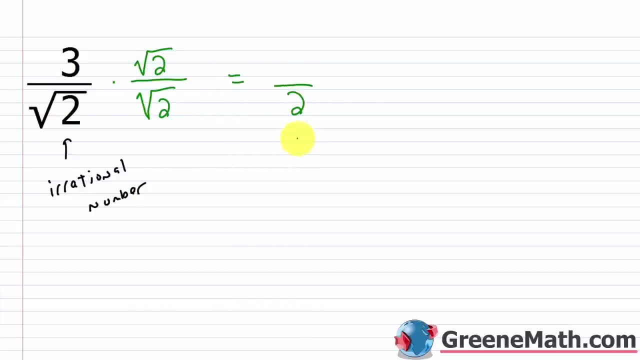 That gives me 2.. So the denominator is now a rational number. Okay, It's a rational number. Henceforth the term rationalizing the denominator. We're taking it from an irrational number and we're making it into a rational number. 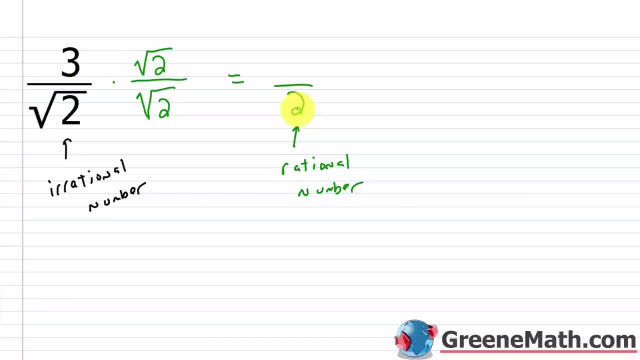 So again, that's rationalizing the denominator. That's where the term comes from. Then I just multiply 3 times the square root of 2.. Can't make that any simpler. I just write 3 times the square root of 2.. 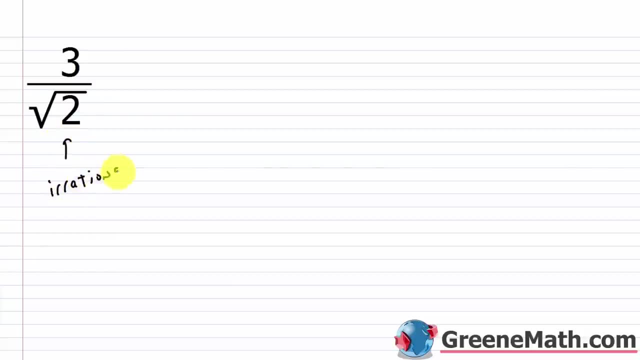 This is an irrational number. We don't want this. So what could we possibly do? Well, if we don't have a radical in the denominator, what could we possibly do to get rid of it? Well, I didn't say that I couldn't have a radical in the numerator. If I just don't want one in the denominator, all I need to do is perform a little trick that we learned back when we studied fractions. I'm going to multiply the denominator by the square root of 2, and I'm going to do the same thing to the numerator. Remember, the square root of 2 over the square root of 2 is a complicated form of 1. Same nonzero number over itself, it's 1. Okay? Now what happens when I'm multiplying the square root of 2 times the square root of 2? That gives me 2. So the denominator is now a rational number. Okay? It's a rational number. Henceforth, the term rationalizing the denominator. We're taking it from an irrational number, and we're making it into a rational number. So again, that's rationalizing the denominator. That's where the term comes from. Then I just multiply 3 times the square root of 2. Can't make that any simpler. 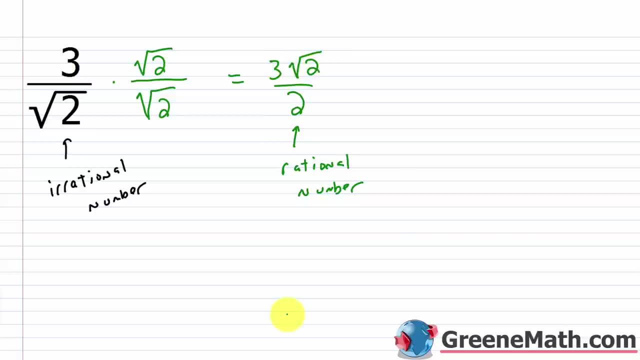 I just write 3 times the square root of 2. Now, the value of this and this is the same. Punch it up on a calculator, you're going to get the same irrational number, but it's just considered simplified to have it in this format versus this one. All right, let's jump through and look at some examples here. And there's some 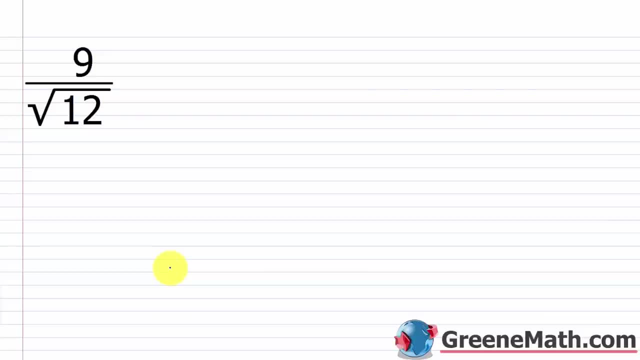 tricks that you need to know when you're dealing with this. It's a very simple process overall. 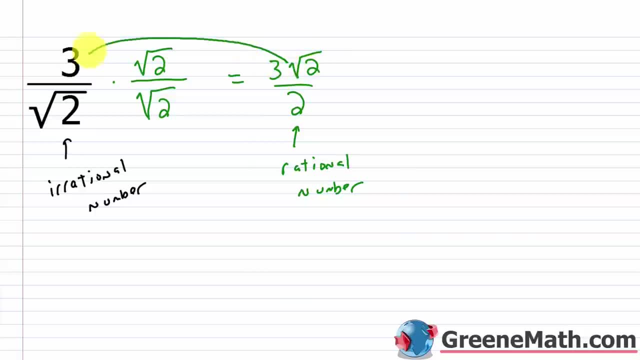 Now the value of this. and this is the same. Punch it up on a calculator. You're going to get the same irrational number. But it's just considered simplified to have it in this format versus this one. All right, Let's jump through and look at some examples here. 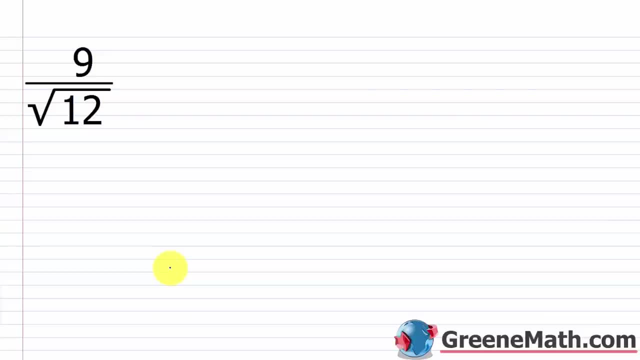 And there's some tricks that you need to know when you're dealing with this. It's a very simple process overall. So let's say I saw something like 9 over the square root of 2.. Do I want to just say, okay, I'm going to multiply this by square root of 12 over square root of 12?? 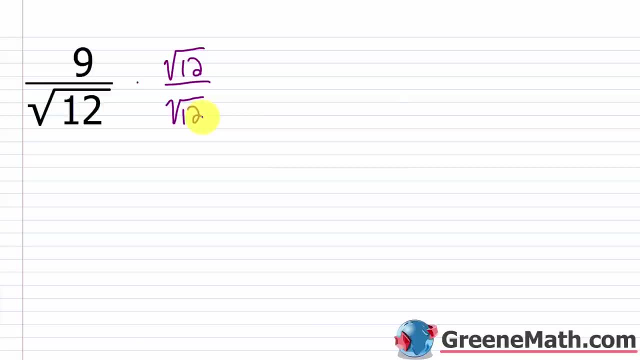 Yes, I can do that, But I'm going to show you in a minute that there's an easier way to do it. So this times this would give me 12.. Right, Square root of 12 times square root of 12 is 12.. 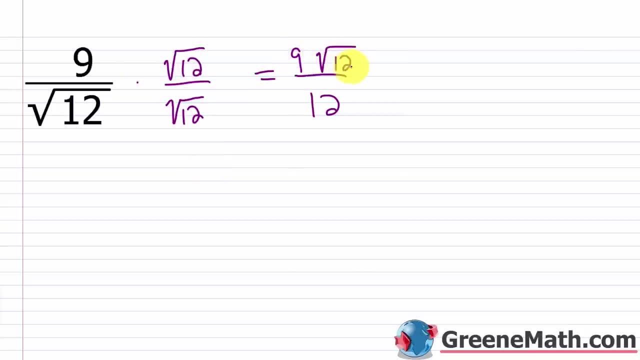 And then I have 9 times square root of 12.. The problem is here. I can simplify the square root of 12. Right One of its factors is a perfect square. Right 4 is, So I can really write this as 9 over the square root of 12.. 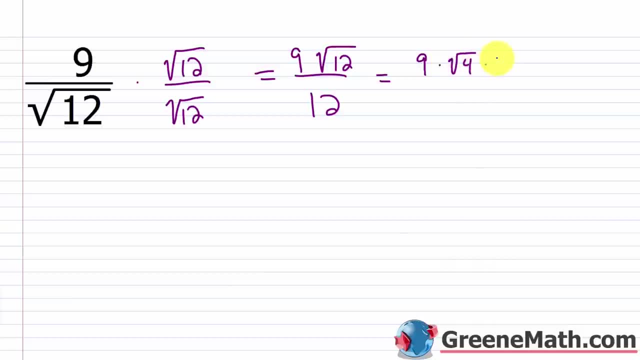 So I can really write this as 9 times the square root of 4 times the square root of 3 over 12.. I know that the square root of 4 is 2.. So let's erase this and just put a 2 here. 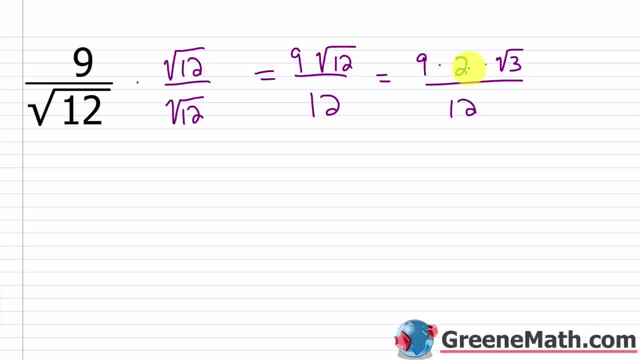 Now between the numerator and denominator. I could do some canceling, Right, If I think about 9 and I think about 12, they each share a factor of 3.. So let's cancel this with this and put a 3 here and a 4 here. 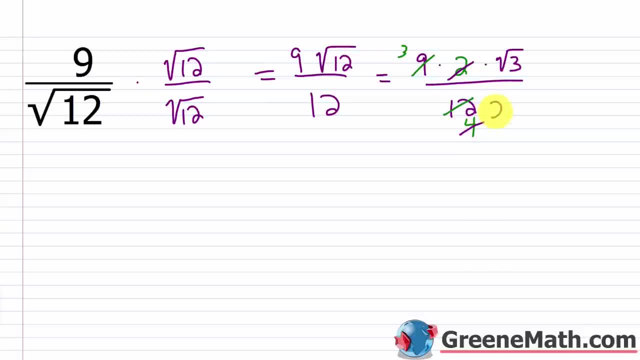 And then let's cancel between the 2 and the 4. And leave a 2. And basically I'm going to have a 3 times the square root of 3 in the numerator over a 2 in the denominator, So 3 times the square root of 3 over 2.. 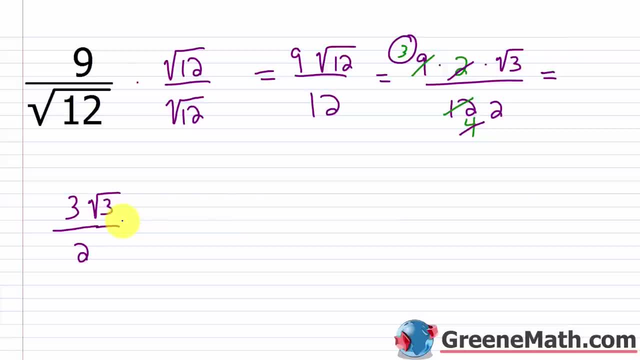 Now you can do it that way. We've rationalized the denominator, We've reported a simplified radical. But there's an easier way to kind of look at this. Let's say I erase this and start the problem over What if? before I begun. 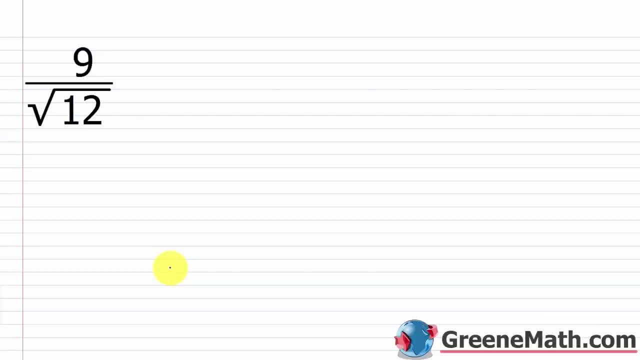 So let's say I saw something like 9 over the square root of 12. Do I want to just say, I'm going to multiply this by square root of 12, over square root of 12? Yes, I can do that. But I'm going to show you in a minute that there's an easier way to do it. So this times this would give me 12, right? Square root of 12 times square root of 12 is 12. And then I have 9 times square root of 12. The problem is here, I can simplify the square root of 12, right? One of its factors is a perfect square, right? 4 is. So I can really write this as 9 times the square root of 4 times the square root of 3 over 12. I know that the square root of 4 is 2. So let's erase this and just put a 2 here. Now, between the numerator and denominator, I can do some canceling, right? If I think about 9 and I think about 12, they each share a factor of 3. So let's cancel this with this and put a 3 here and a 4 here. And then let's 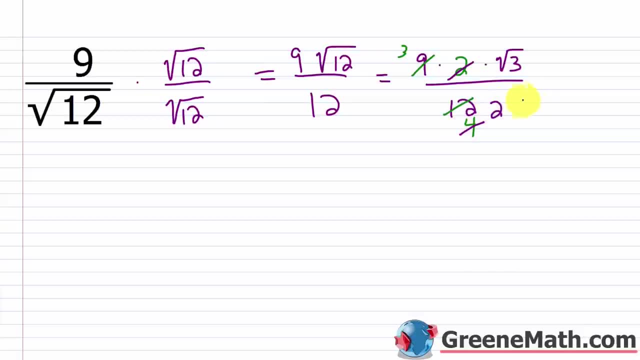 cancel between the 2 and the 4 and leave a 2. And basically, I'm going to have a 3 times the square root of 3 in the numerator. 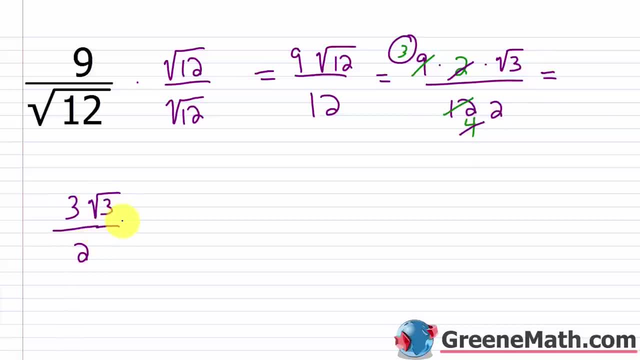 Over a 2 in the denominator. So 3 times the square root of 3 over 2. Now, you can do it that way. 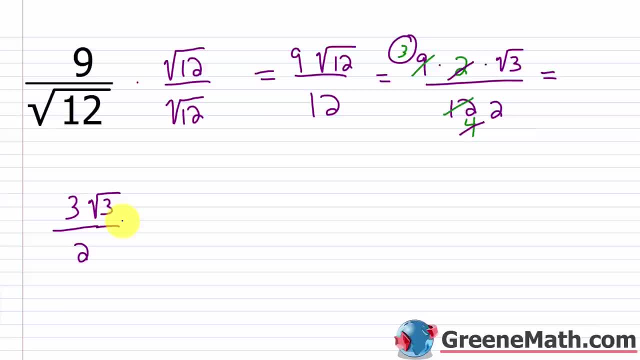 We've rationalized the denominator. We've reported a simplified radical. But there's an easier way to kind of look at this. Let's say I erase this and start the problem over. What if before I begun, I simply said, okay, this is the square root of 12. Now, I know that 12 has a perfect square 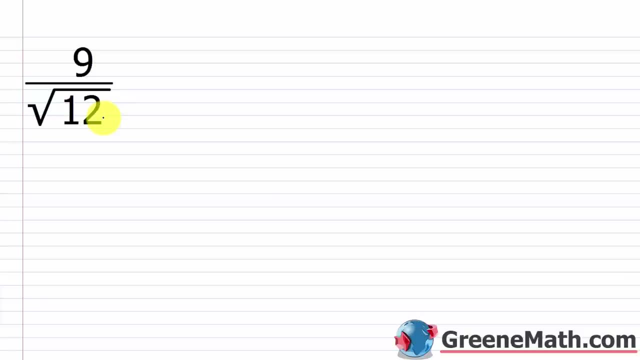 root of 4. So let's put 9 over the square root of 4 times the square root of 3. And I know the square root of 4 is 2. So let's just put 2 times the square root of 3. Now, because this right here is a rational number, I don't really need to worry about it. All I need to worry about is this irrational number, this square root of 3. So when I'm over here, I'm going to put 9 over the square root of 4. 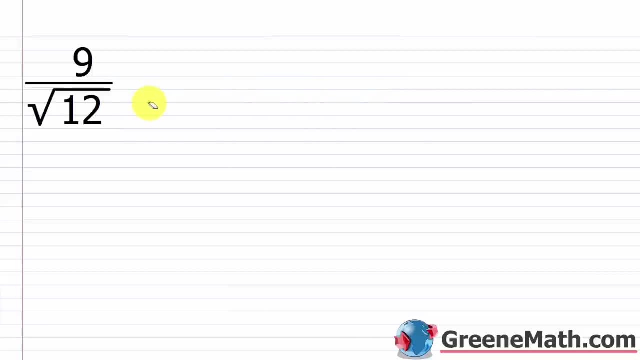 I simply said: okay, this is the square root of 12.. Now I know that 12 has a perfect square involved in it: Square root of 4.. If I simplify that before I begin, it's going to lessen my work. 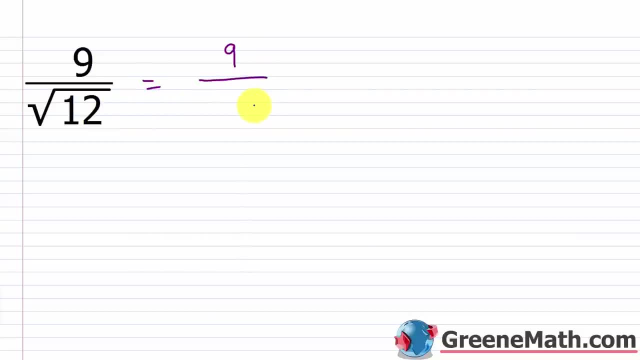 So let's put equals 9 over. I can say square root of 4 times square root of 3.. And I know the square root of 4 is 2.. So let's just put 2 times the square root of 3.. 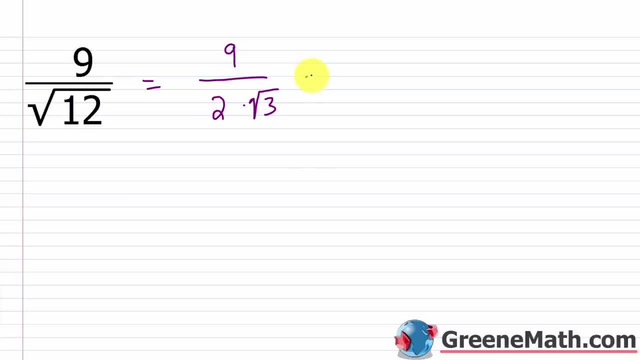 Now, Because this right here is a rational number, I don't really need to worry about it. All I need to worry about is this irrational number, This square root of 3.. So when I multiply now, I'm just going to multiply the numerator and denominator by the square root of 3.. 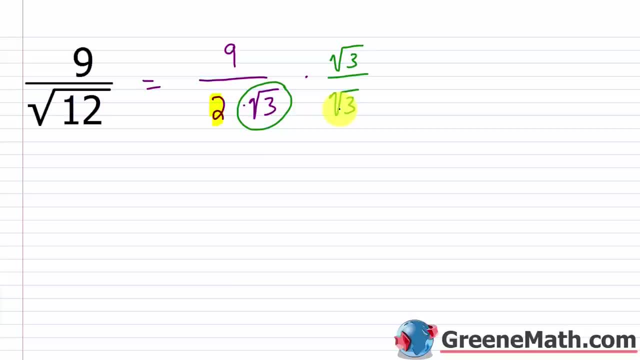 And what's going to happen is: Square root of 3 times square root of 3 is 3.. So that's 3.. And then you still have your 2 there, So 2 times 3.. Let me just write it like this: 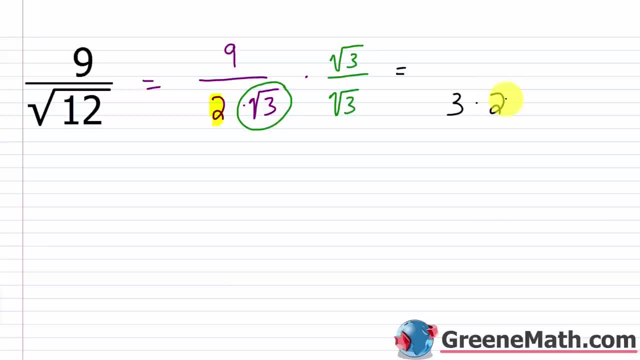 Would give you 6.. I'm not going to write that out, because there's some things we can cancel, obviously. And then we have 9 times square root of 3.. So 9 times square root of 3. And then this will cancel with this and give me a 3.. 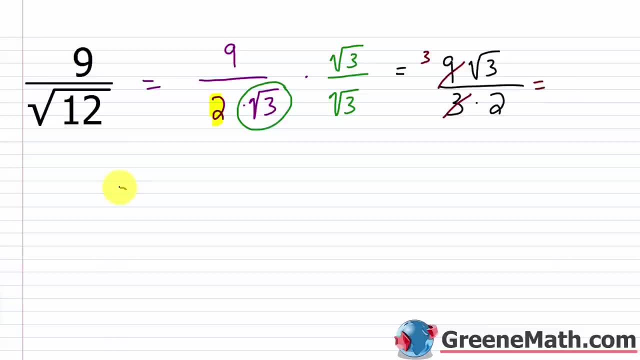 So kind of. either way I do that I end up with 3 times square root of 3 over 2.. But I feel like if you simplify before you begin, If you just attack the problem and simplify before you just start jumping in there. 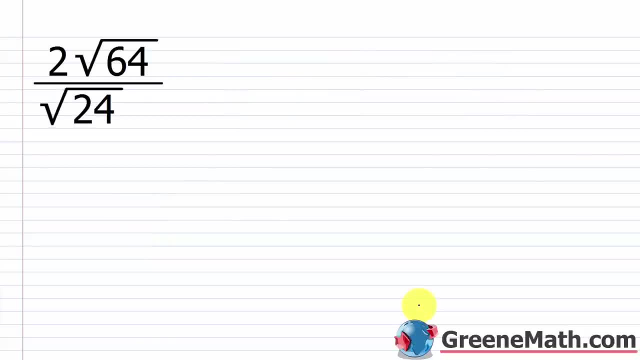 You end up with less work in the end. Alright, Let's take a look at another one. So we have 2 times the square root of 64 over the square root of 24.. So let's simplify. So we have 2 times. 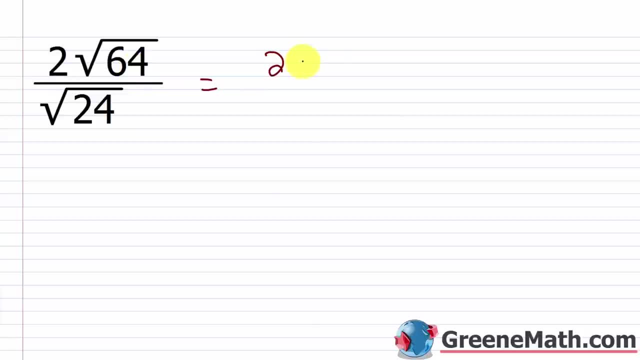 The square root of 64 is 8.. Right, We should know that at this point. So, 2 times 8 over The square root of 24, I'm going to write as the square root of 4 times the square root of 6.. 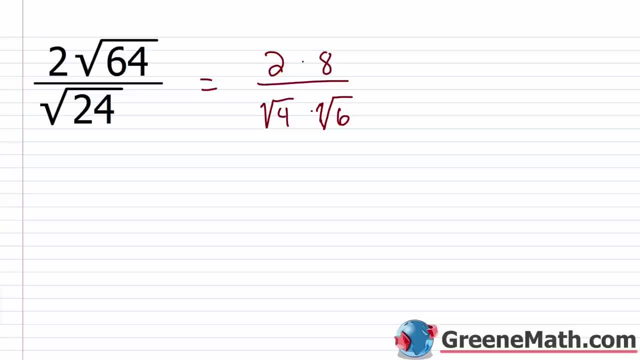 Now the square root of 4 is 2.. So, without even doing that, I know I can cancel this with this. Square root of 4 and 2 are the same, So that's gone. So really, what I have here is 8 over the square root of 6.. 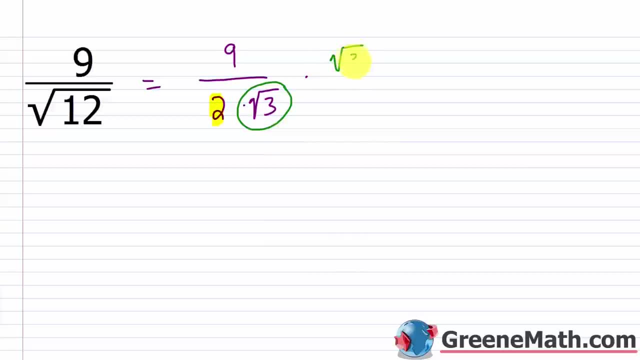 Multiply now. I'm just going to multiply the numerator and denominator by the square root of 3. And what's going to happen is square root of 3 times square root of 3 is 3. So that's 3. And then you still have your 2 there. So 2 times 3, let me just write it like this, would give you 6. I'm not going to write that out because there's some things we can cancel, obviously. And then we have 9 times square root of 3. So 9 times square root of 3. And then this will cancel with this and give me a 3. So kind of either way, I'm going to put 9 over the square root of 3. And then I'm going to put 9 over the 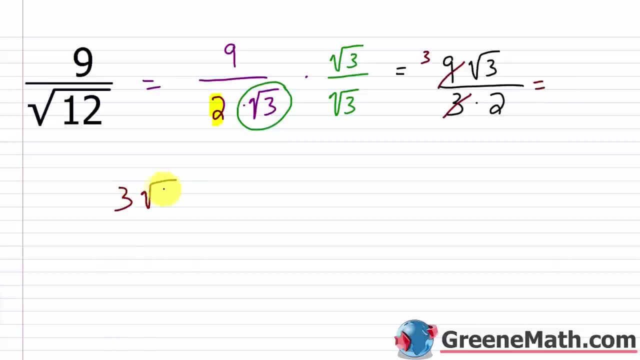 denominator. So this is the usual way I do that. I end up with 3 times square root of 3 over 2. But I feel like if you simplify before you begin, if you just attack the problem and simplify before, 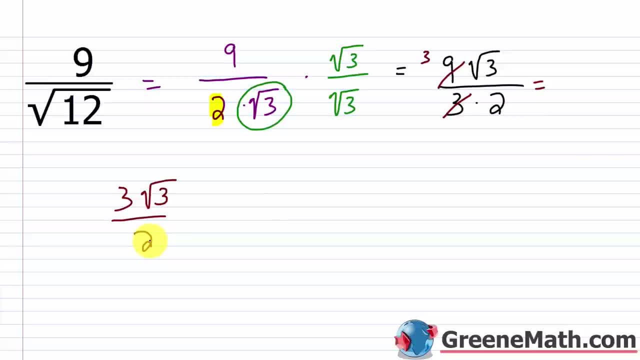 you know, you just start jumping in there, you end up with less work in the end. All right, let's take a look at another one. So we have 2 times the square root of 64 over the square root 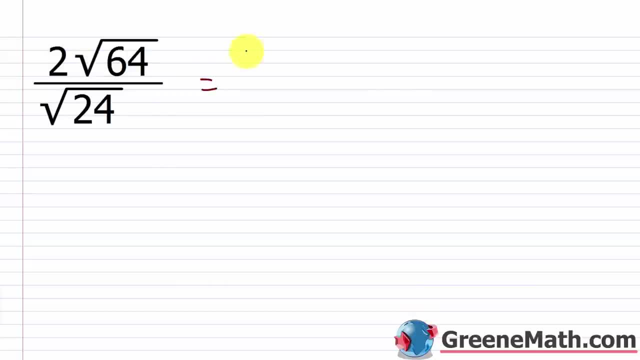 of 24. So let's simplify. So we have 2 times, the square root of 64 is 8, right? We should know that at this point. So let's simplify. So we have 2 times, the square root of 64 is 8, right? We should know that at this point. 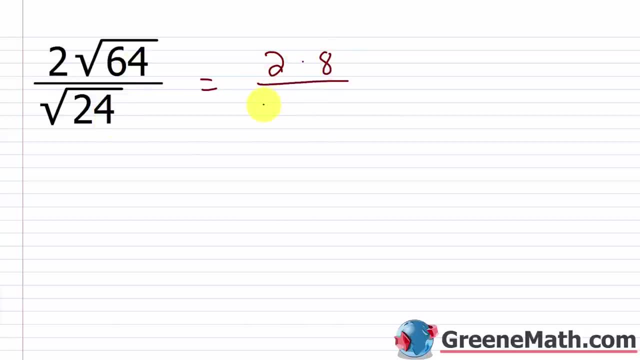 So 2 times 8 over the square root of 24, I'm going to write as the square root of 4 times the square root of 6. 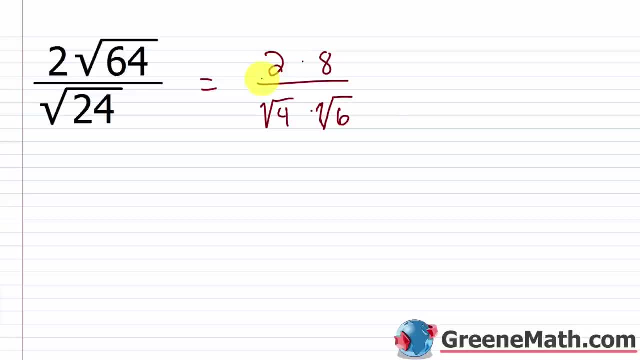 Now the square root of 4 is 2, so without even doing that, I know I can cancel this with this. The square root of 4 and 2 are the same, so that's gone. 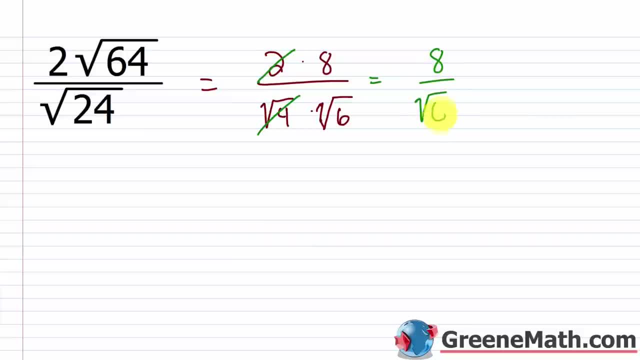 So really what I have here is 8 over the square root of 6, and I'm simply going to multiply the numerator and denominator by the square root of 6, and that's going to give me what? I'll have 8 times the square root of 6 over the square root of 6 times the square root of 6 is 6, and then I can cancel one factor of 2 between numerator and denominator, that's 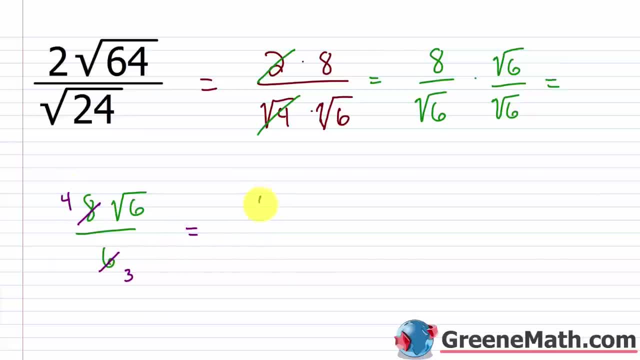 going to give me a 4 here and a 3 here, and so I'm going to end up with 4 times the square root of 6 over 3 as my simplified answer. 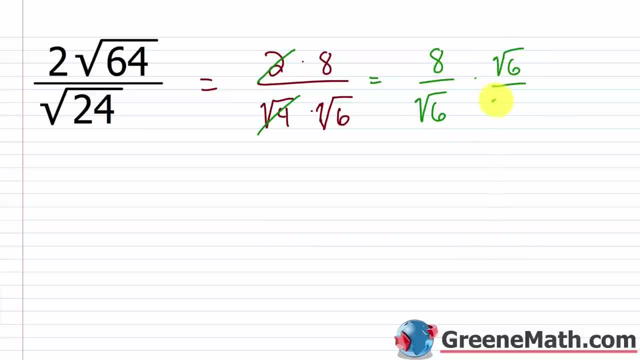 And I'm simply going to multiply the numerator and denominator by the square root of 6.. And that's going to give me what I'll have: 8 times the square root of 6 over Square root of 6 times the square root of 6 is 6.. 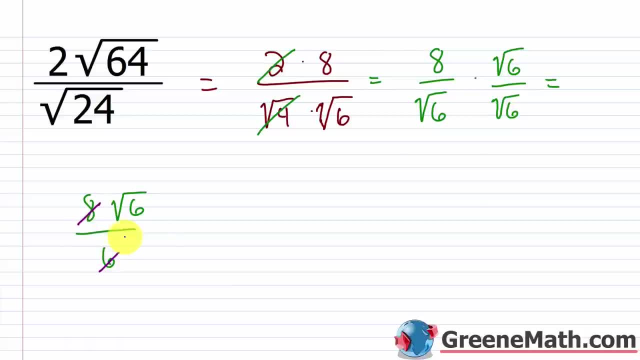 And then I can cancel 1 factor of 2 between numerator and denominator. That's going to give me a 4 here and a 3 here, And so I'm going to end up with 4 times the square root of 6.. 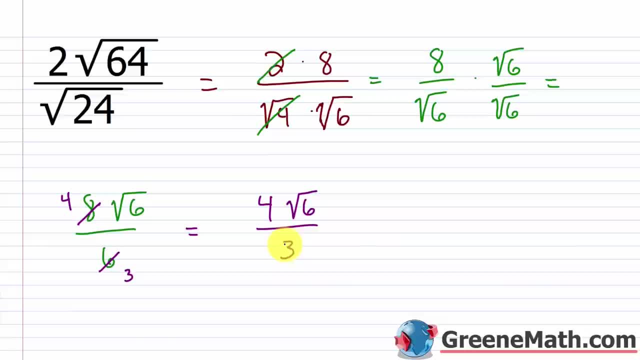 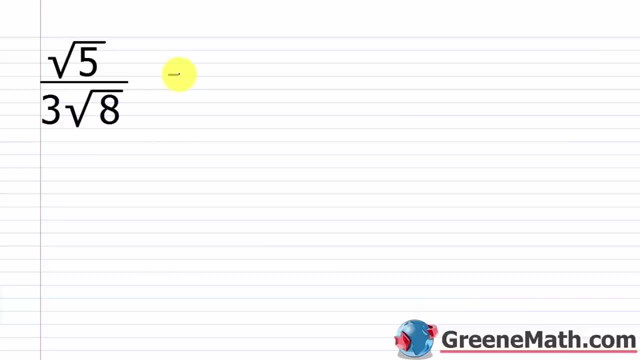 So square root of 6 over 3 is my simplified answer. Alright, let's take a look at square root of 5 over 3 times the square root of 8.. Again, we want to simplify before we begin. So I know square root of 5.. 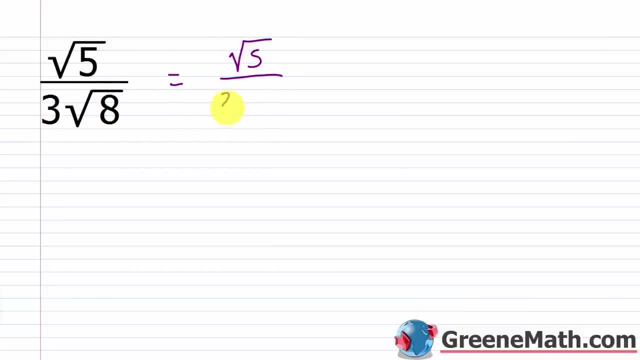 I can't do anything with that. 3 times the square root of 8.. I know the square root of 8 at this point is the square root of 4 times the square root of 2.. So, square root of 4 times the square root of 2.. 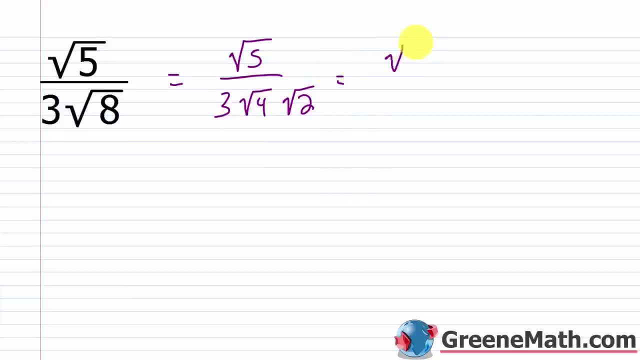 Then I know this is 2 right here. So let's write this as the square root of 5 over 3 times 2 would be 6.. So 6 times the square root of 2.. And now all I need to do is multiply the numerator and denominator here by the square root of 2.. 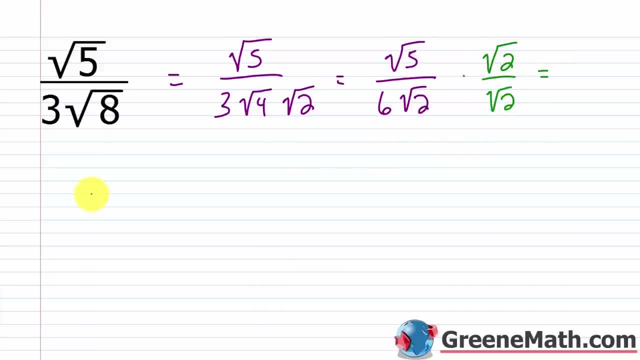 So the square root of 5 times the square root of 2 is square root of 10 over We have 6 times the square root of 2 times the square root of 2 times the square root of 2 is 2.. 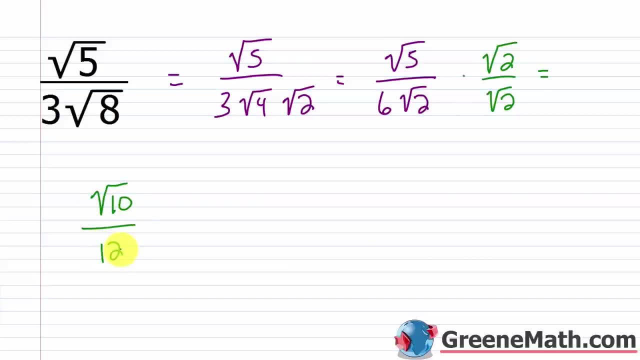 2 times 6 would be 12.. So I get the square root of 10 over 12.. And again, that is as simple as you can make that. What about something like the square root of 3 over the square root of 7.? 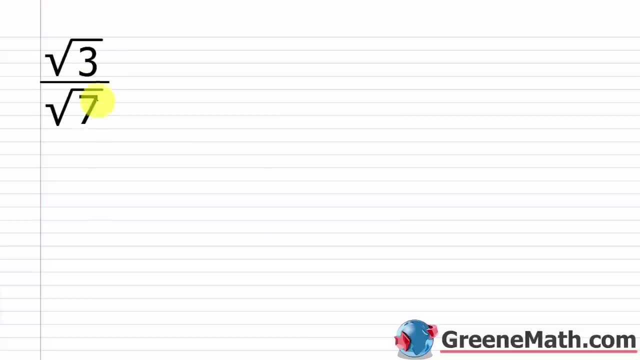 So I can't simplify either of these. So basically, all I'm going to do is look at my denominator. If I have the square root of 7 there, I'm going to multiply by the square root of 7 over the square root of 7.. 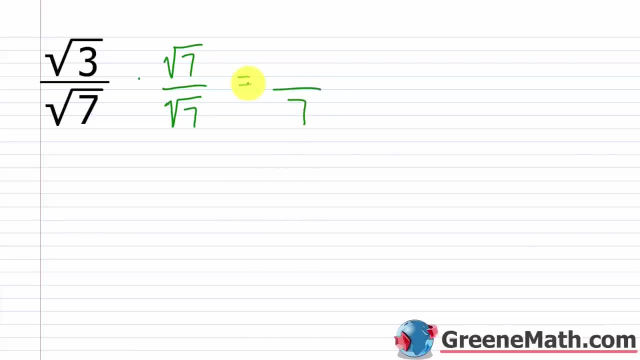 Square root of 7 times square root of 7 is 7.. Square root of 3 times square root of 7 is square root of 21.. So I get square root of 21 over 7.. What about something like the square root of 48 over the square root of 42?? 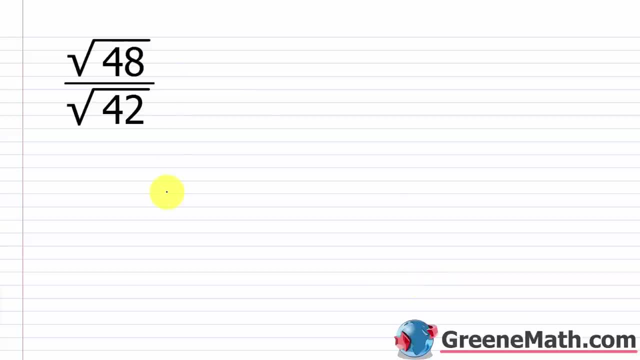 Again, I want to simplify before I kind of start rationalizing the denominator. A lot of students just jump right in and go: okay, I want to do square root of 42 over square root of 42. That's going to give you more work in the end. 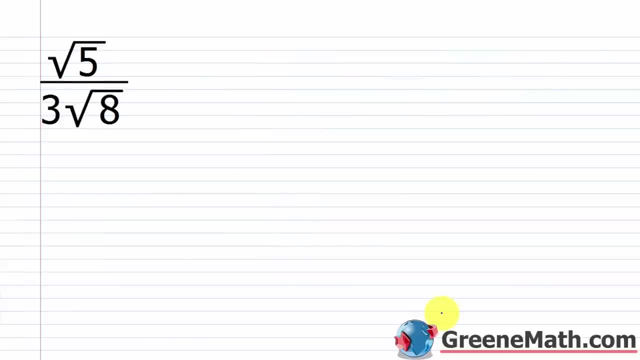 Alright, let's take a look at square root of 5 over 3 times the square root of 8. Again, we want to simplify before we begin, so I know square root of 5, I can't do anything with that. 3 times the square root of 8, I know the square root of 8 at this point is the square root of 4 times the square root of 2, so square root of 4 times the square root of 2, then I know this is 2 right here, so let's write this as the square root of 5 over 3 times 2 would be 6, so 6 times the square root of 2, and now all I need to do is multiply the numerator and denominator here by the square root of 2. So the square root of 5 times the square root of 2 is the square root of 10. 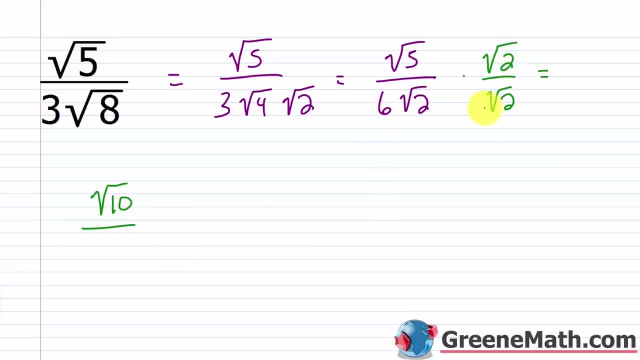 Over, we have 6 times the square root of 2 times the square root of 2. Square root of 2 times the square root of 2 is 2, 2 times 6 would be 12, so I get square root of 10 over 12, and again that's as simple as you can make that. 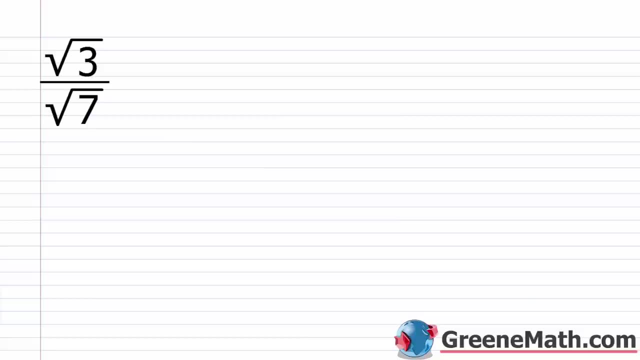 What about something like the square root of 3 over the square root of 7? So I can't simplify either of these, so basically all I'm going to do is look at my denominator. If I have the square root of 7 there, I'm going to multiply by the square root of 7 over the square root of 7. Square root of 7 times the square root of 7 is 7. Square root of 3 times the square root of 7 is square root of 21. 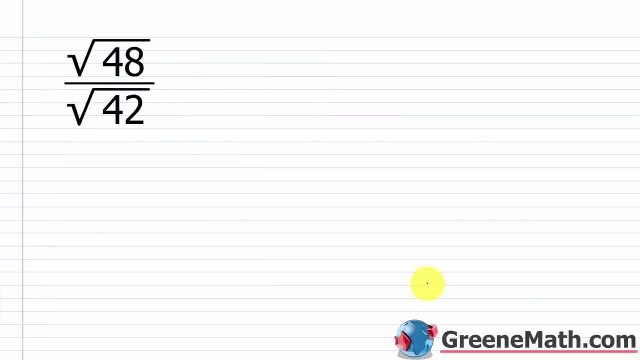 So I get square root of 21 over 7. What about something like the square root of 48 over the square root of 42? 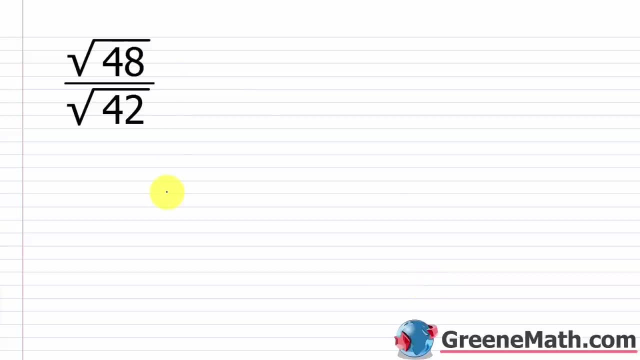 Again, I want to simplify before I kind of start rationalizing the denominator. A lot of students just jump right in and go, okay, I want to do square root of 42 over square root of 42. That's going to give you more work in the end. 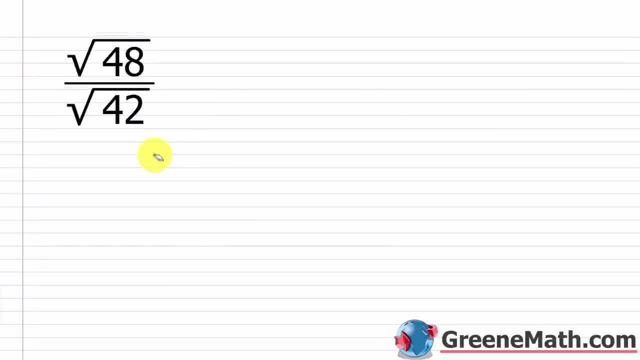 You don't want to do that. So let's see if we can simplify this. 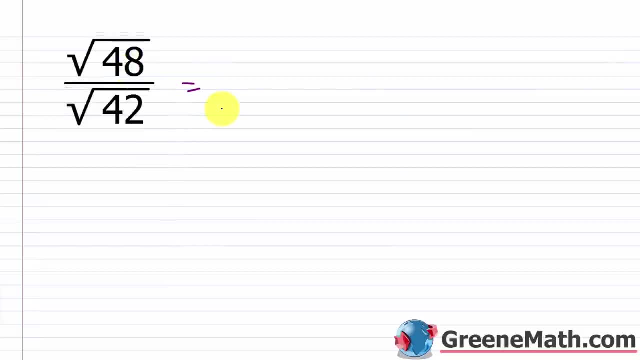 So square root of 48, I know 48 is 16 times 3. 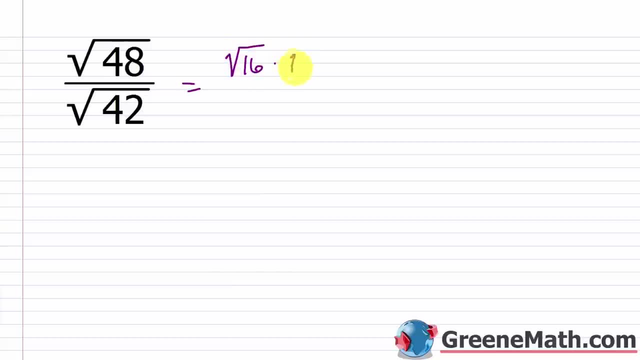 So 16 is a perfect square. So we do square root of 16 times square root of 3. 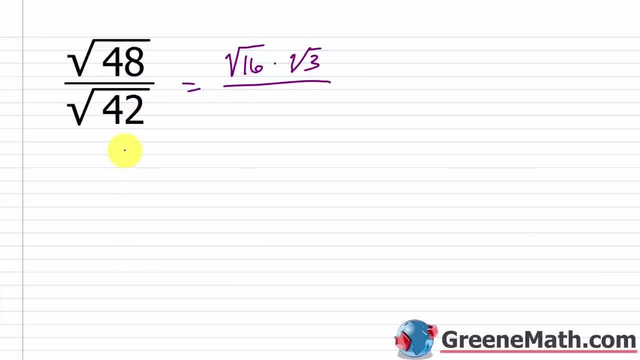 And for 42, I know 42 is 7 times 2 times 3. So no perfect squares in there. I got a 7, I got a 2, and I got a 3. 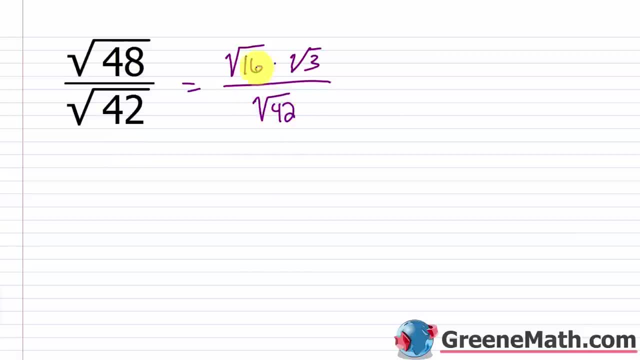 So really it's just square root of 42, just square root of 42. So this right here, I can simplify. I know that would be 4. So this becomes 4 times square root of 3. 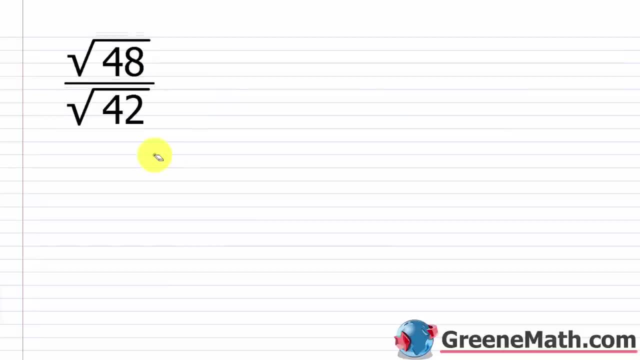 You don't want to do that. So let's see if we can simplify this. So square root of 48, I know 48 is 16 times 3.. So 16 is a perfect square. So we do square root of 16 times square root of 3.. 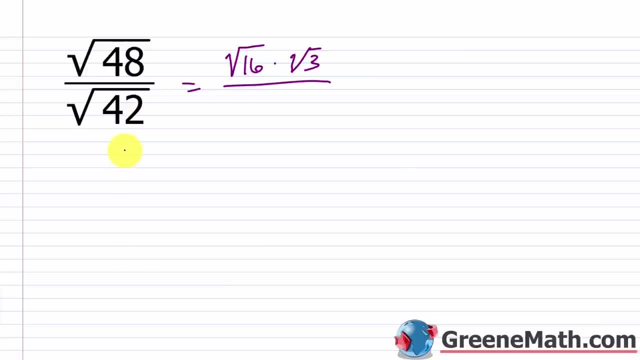 And for 42.. I know 42 is 7 times 2 times 3.. So no perfect squares in there. I got a 7, I got a 2, and I got a 3.. So really it's just square root of 42.. 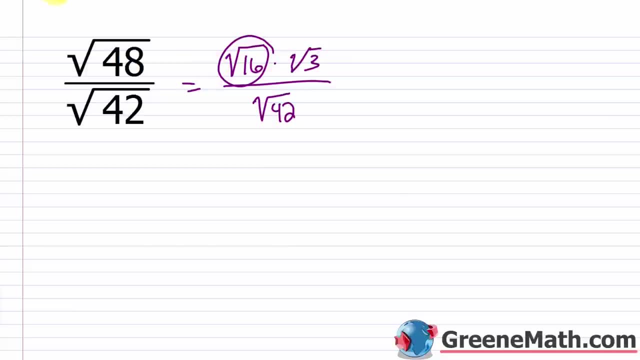 Just square root of 42. So this right here I can simplify. I know that would be 4.. So this becomes 4 times square root of 3 over the square root of 42. So now we're just going to multiply the numerator and denominator by that square root of 42.. 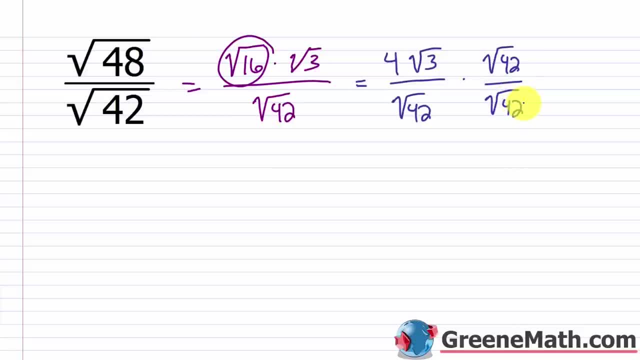 And I know we end up doing that. So you might say, well, why did you go? Why did you go through all the process of, you know, trying to simplify it? It just saves yourself a lot of work in the end. 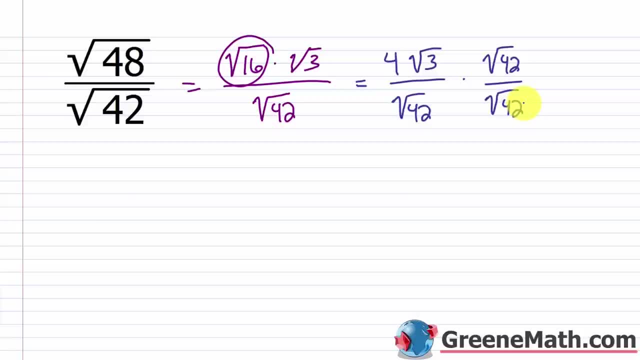 You just want to take that extra time and try to simplify, Because even reducing this a little bit is going to knock some of your workload down. So if I have the square root of 42 times square root of 42, I know that's going to be equal to 42.. 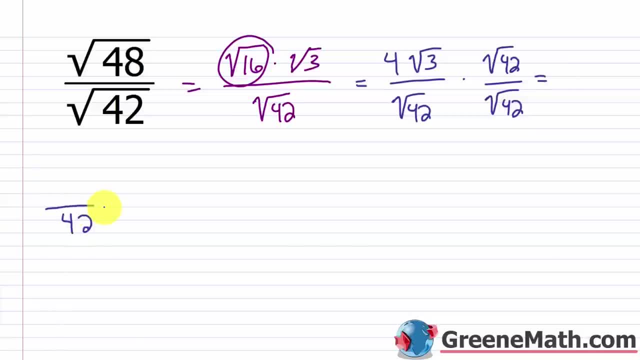 So that's my denominator. For my numerator, I'm going to have 4 times the square root of 3 times the square root of 42.. Now, 3 times 42 is 125.. But if I think about 126,, I want you to remember that 42 was what. 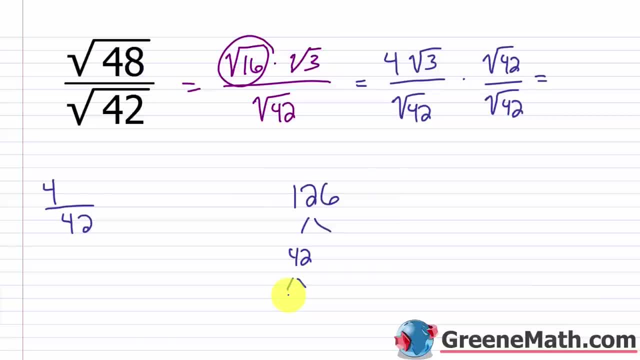 42 was 7 times 2 times 3.. So you're going to have a perfect square involved in this. It's going to be 9.. So I can think about this as 42 times 3.. 42 again is 7 times 6.. 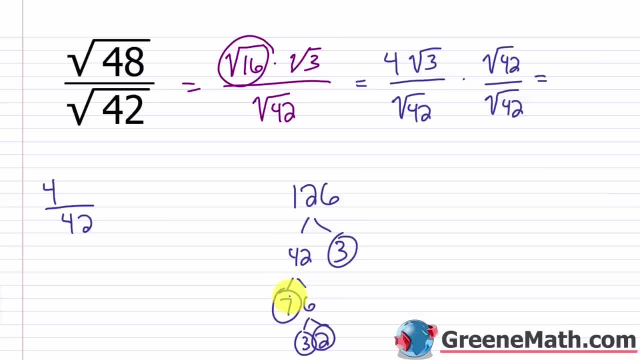 6 is 3 times 2.. So I can really think about this as 14 times 9.. So let's write this as the square root of 42.. Let's write this as the square root of 42.. Let's write this as the square root of 14 times the square root of 9.. 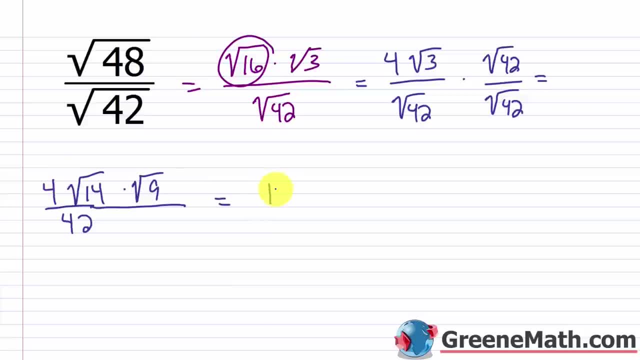 And then the square root of 9 is 3.. So 3 times 4 would be 12.. I'll have 12 times the square root of 14 over 42.. And then I've still got some more simplifying to do. 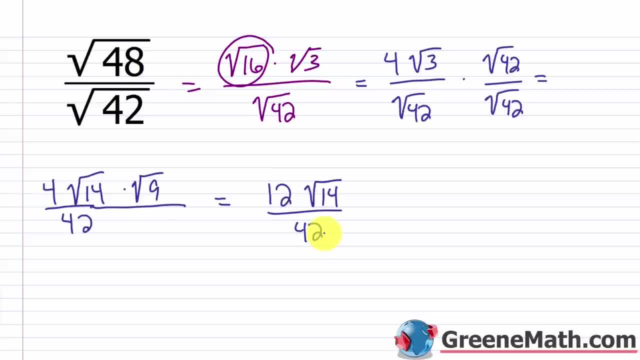 12 and 42 share a common factor of 6.. So 12 divided by 6 would be 2.. 42 divided by 6 would be 7.. So in the end, my simplified form is going to be 2 times 6.. I know that would be 4. So this becomes 4 times square root of 3. 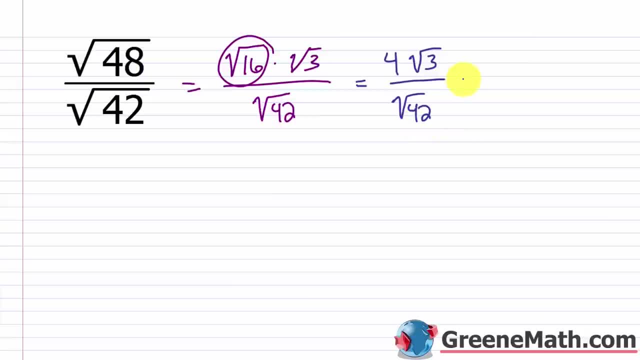 Over the square root of 42. So now we're just going to multiply the numerator and denominator by that square root of 42. 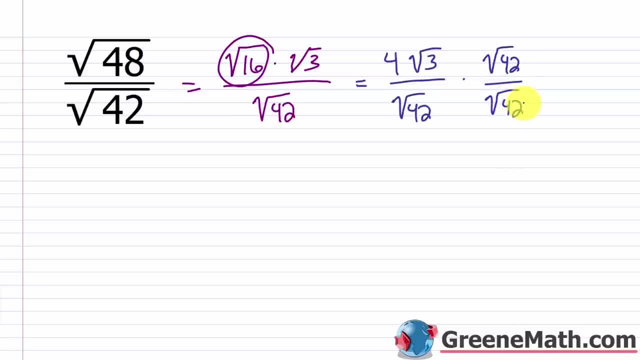 And I know we end up doing that. So you might say, well, why did you go through all the process of trying to simplify it? It just saves yourself a lot of work in the end. You just want to take that extra time and try to simplify because even reducing this a little bit is going to knock some of your workload down. 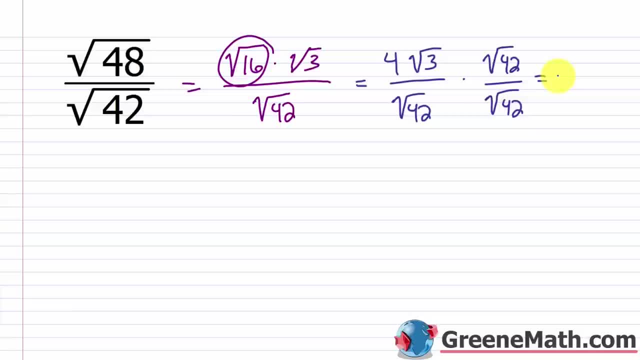 So if I have the square root of 42 times the square root of 42. I know that's going to be equal to 42. 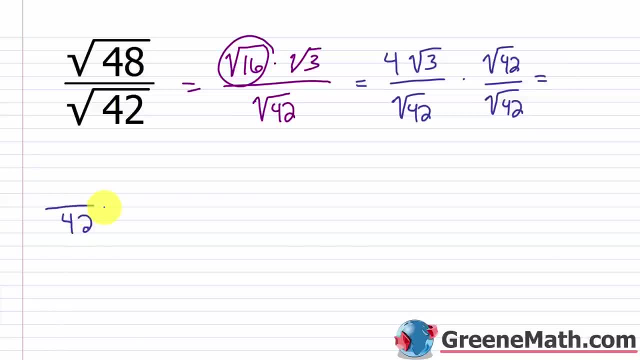 So that's my denominator. For my numerator, I'm going to have 4 times the square root of 3 times the square root of 42. 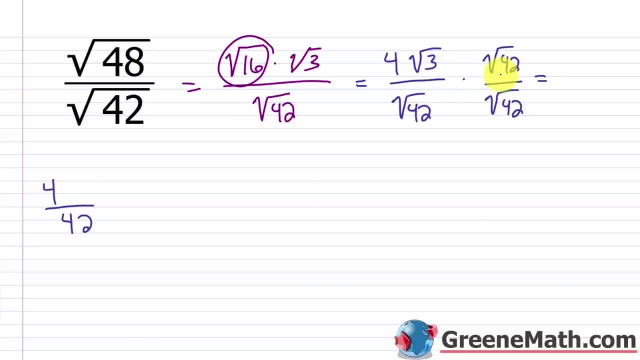 Now 3 times 42 is 126. But if I think about 126, I want you to remember that 42 was what? 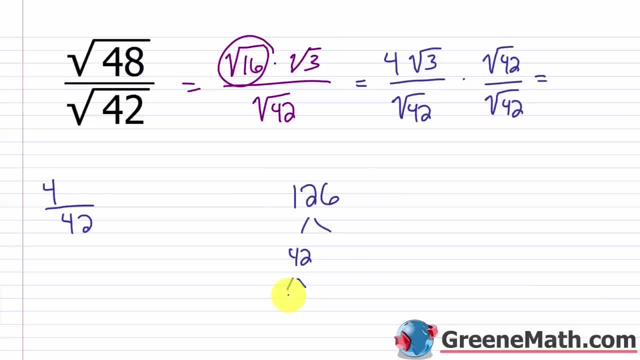 42 was 7 times 2 times 3. So you're going to have a perfect square involved in this that's going to be 9. So I can think about this as 42 times 3. 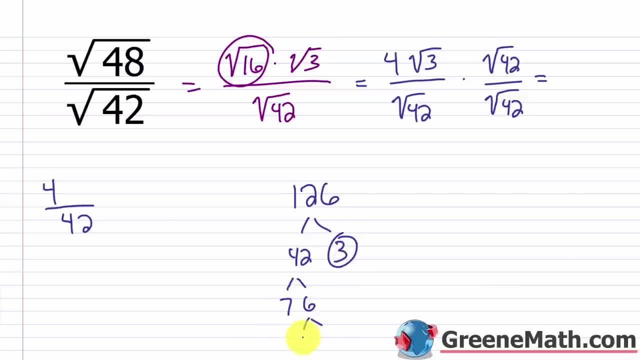 three. Forty-two again is seven times six. Six is three times two. So I could really think about this as fourteen times nine. So let's write this as the square root of fourteen times the square 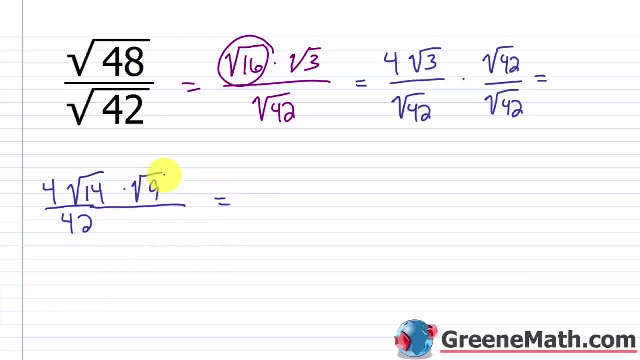 root of nine. And then the square root of nine is three. So three times four would be twelve. 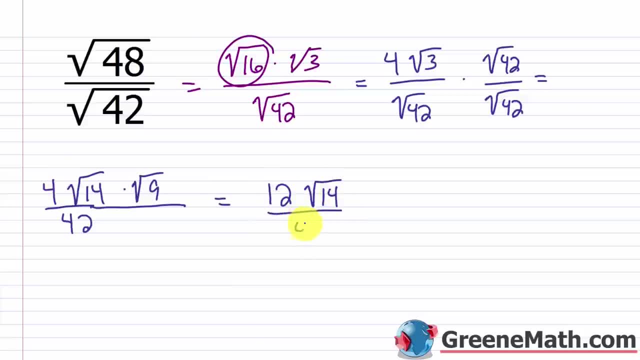 I'll have twelve times the square root of fourteen over forty-two. And then I've still got some more simplifying to do. Twelve and forty-two share a common factor of six. So twelve divided by six 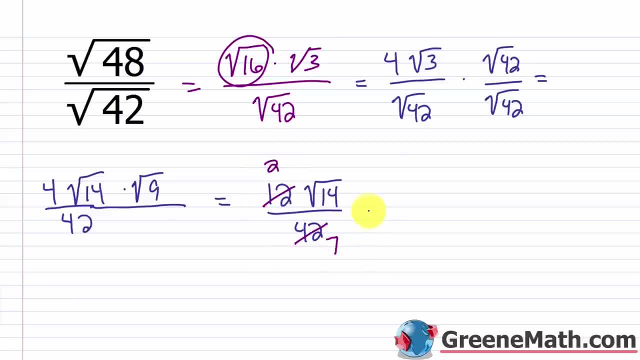 would be two. Forty-two divided by six would be seven. So in the end, my simplified form is going 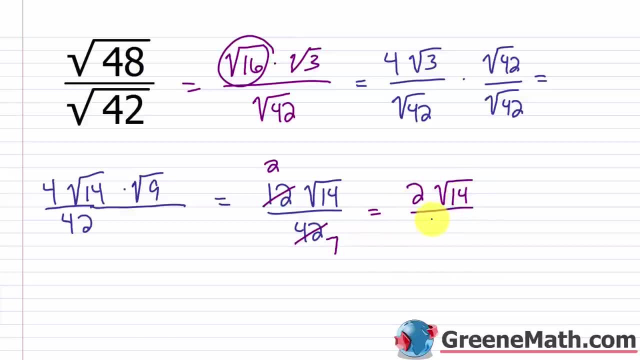 to be two times the square root of fourteen over seven. And again, lots of different ways to kind 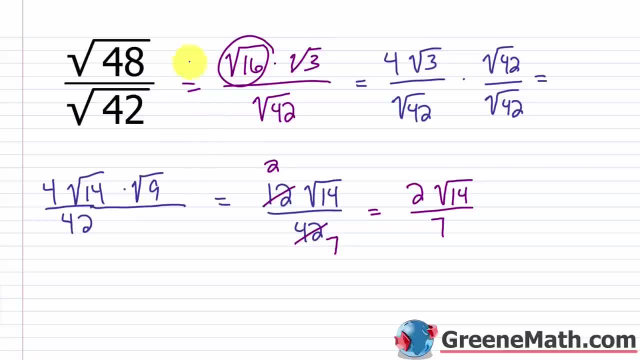 of attack these problems. If you wanted to start out by saying, okay, times square root of forty-two 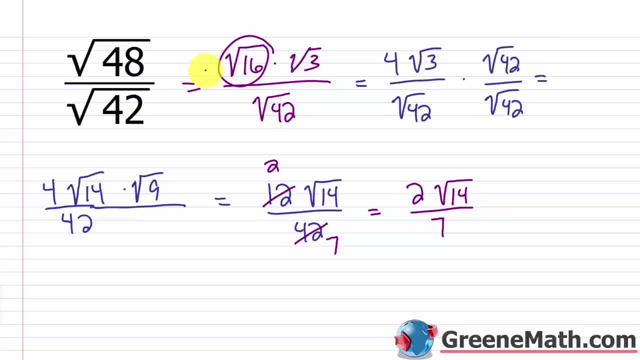 over square root of forty-two, that's fine. You can do that. But I really think if you spend the 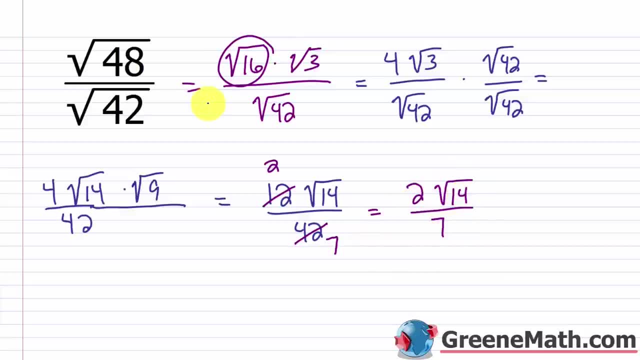 2 times 6 is the square root of 14 over 7.. And again, lots of different ways to kind of attack these problems. If you wanted to start out by saying: okay, times square root of 42 over square root of 42,. 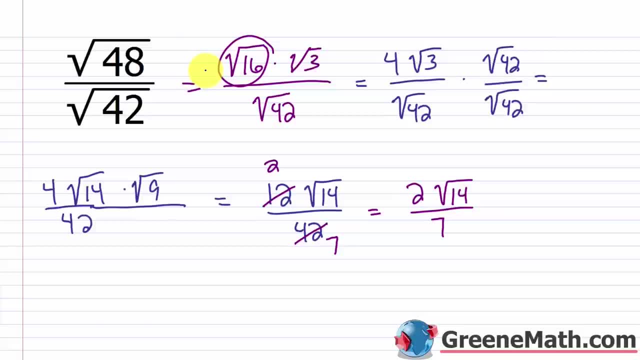 that's fine, You can do that. But I really think if you spend the extra time to try to simplify in the beginning, it saves you work in the end. All right, So now that we've kind of gone through the basic scenarios. 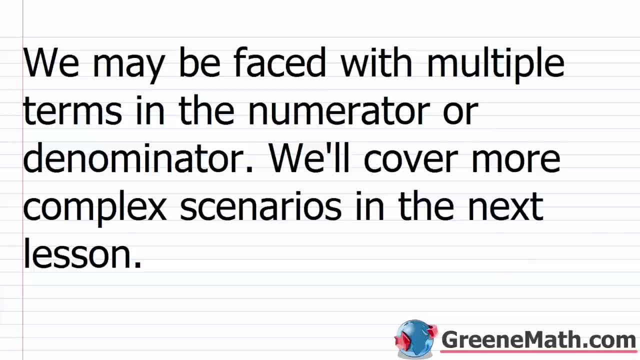 and this isn't a very difficult topic. right, We've kind of blown through those. We may be faced now with multiple terms in the numerator or denominator, And we'll cover more complex scenarios in the next lesson. We're going to do a lesson called further operations with radicals. 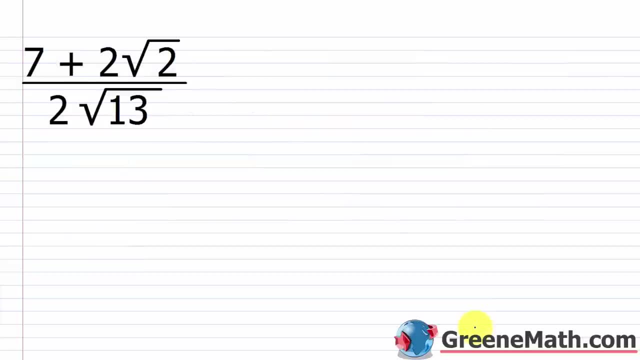 And we're going to cover some more complex scenarios there. So what if you saw something like 7 plus 2 times the square root of 2 over 2 times the square root of 13?? Well, this is already pretty well simplified, right. 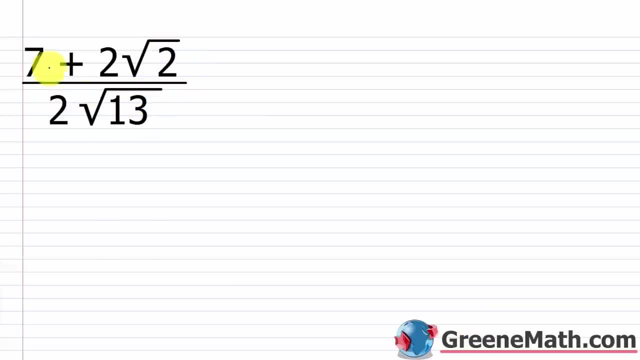 I can't do anything with square root of 13.. Can't do anything with square root of 2.. Can't add here because I don't have like radicals. So what am I going to do? Well, all I need to do is. 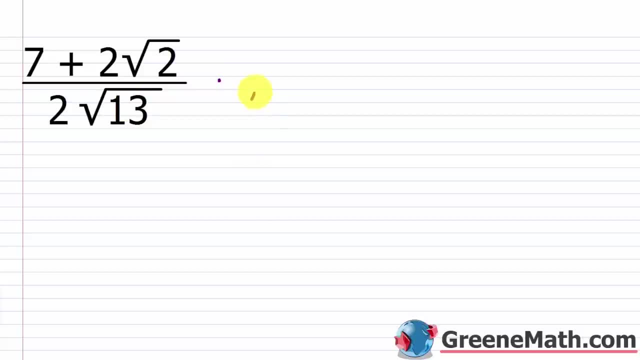 is: multiply the denominator here by the square root of 13.. If I do that, I'm going to rationalize the denominator, But I've got to do it to the numerator as well. Now pay close attention here. The main mistake that students make is they'll just multiply this by one of these terms. 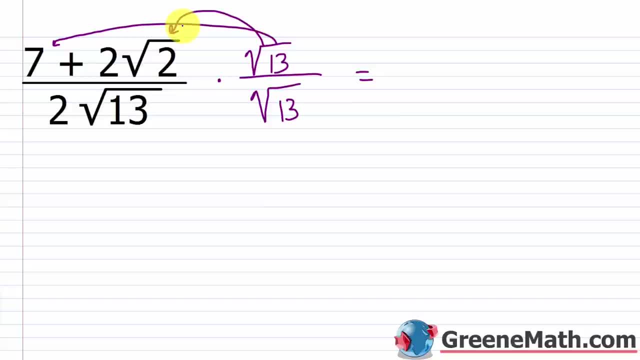 You've got to use the distributive property and multiply this by both terms that are in that numerator. So in other words, I've got to have the square root of 13.. That's multiplied by 7, and then plus the square root of 13.. 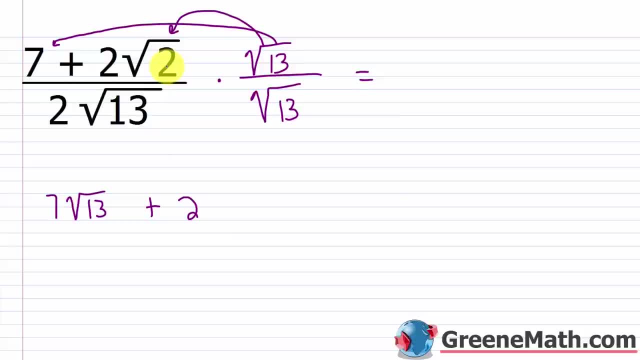 That's multiplied by 2 times the square root of 2.. So square root of 13 times square root of 2 is square root of 26.. So my numerator becomes 7 times square root of 13 plus 2 times the square root of 26.. 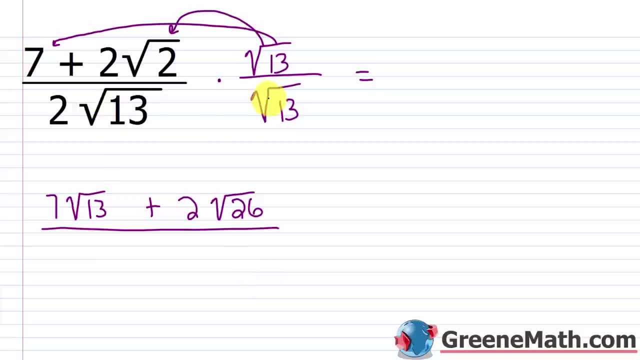 Now, in the denominator, square root of 13 times square root of 13 is 13.. So you're going to have 2 times 13 or 26.. Simplifying is a lot of work. Simplifying is a little bit more challenging here. extra time to try to simplify, 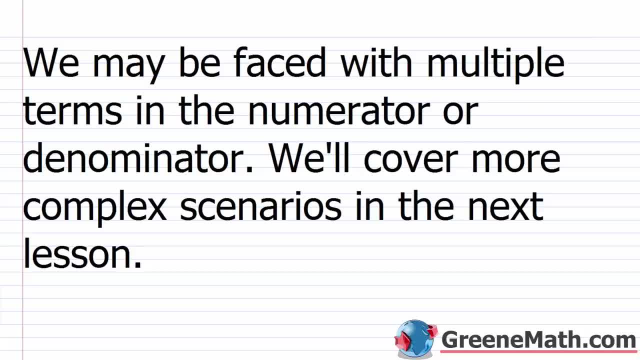 in the beginning, it saves you work in the end. All right. So now that we've kind of gone through the basic scenarios, and this isn't a very difficult topic, right? We've kind of blown through those. We may be faced now with multiple terms in the numerator or denominator. And we'll 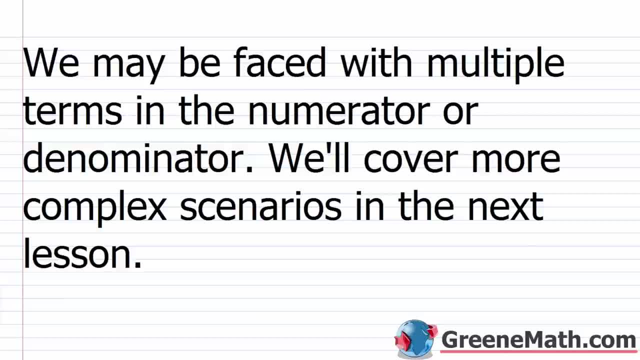 cover more complex scenarios in the next lesson. We're going to do a lesson called further operations with radicals. And we're going to cover some more complex scenarios there. 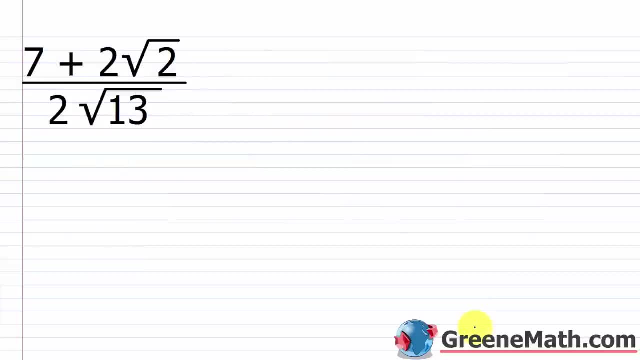 So what if you saw something like seven plus two times the square root of two over twenty-two? 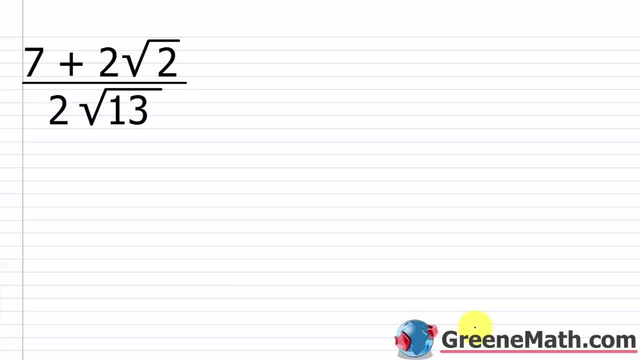 Two times the square root of thirteen. Well, this is already pretty well simplified, right? I can't do anything with the square root of thirteen. Can't do anything with the square root of two. Can't add here because I don't have, like, radicals. So what am I going to do? Well, all I need to do is multiply the denominator here by the square root of thirteen. If I do that, I'm going to rationalize the denominator. But I've got to do it to the numerator as well. Now, pay close attention here. The main mistake that students make 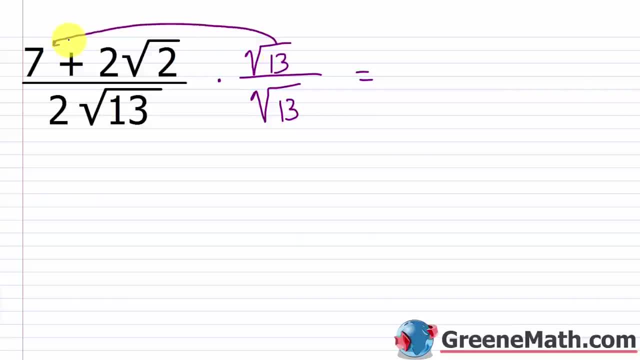 is they'll just multiply this by one of these terms. You've got to use the distributive property and multiply this by both terms that are in that numerator. So in other words, I've got to have the square root of thirteen that's multiplied by seven and plus the square root of thirteen 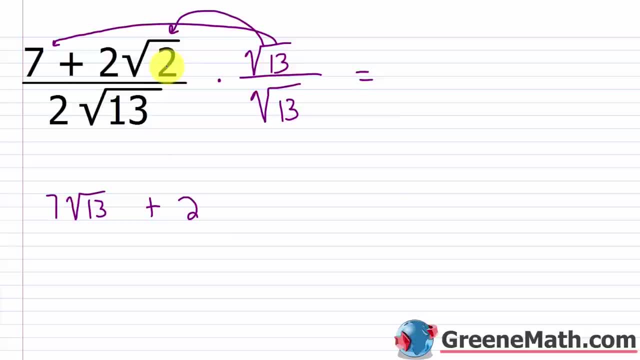 that's multiplied by two times the square root of two. So square root of thirteen times the square root of two is the square root of twenty-six. So my numerator becomes seven 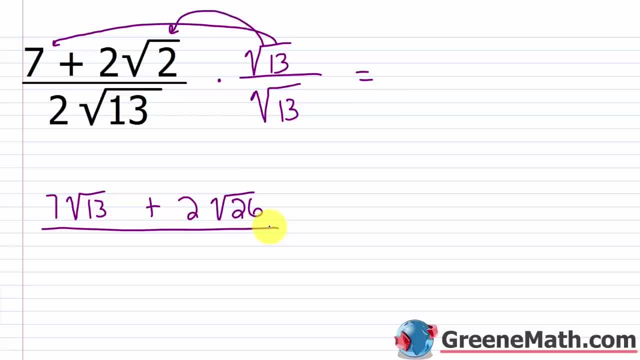 times the square root of thirteen will be being multiplied at that. And then plus 13 at three equals seven times the 13 plus 2 times the square root of 26. Now in the denominator square root of 13 times square root of 13 is 13. So you're going to have 2 times 13 or 26. Simplifying is a little bit more challenging here because remember we can't just go through and cancel stuff. We've got addition. The biggest mistake students make in algebra 1 is they start going through and saying oh I can cancel this with this. This is 13 now. No you can't do that. Remember you cancel common factors. So in order for me to be able to cancel this with something up here I would have to factor something out for it to cancel and there's nothing that's common that I'm going to be able to factor out. I can't factor out a 2. This is a 7. This is a 2. So there's not really anything I'm going to be able to do to simplify this further. I just report my answer at this point and say I have 7 times the square root of 13. 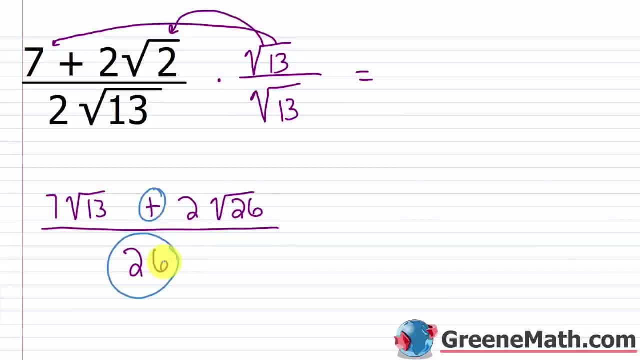 Plus 2 times square root of 26. And this is over 26. What about if we come across negative 2 plus the square root of 6. And this is over the square root of 22. Again if I look at my problem and I don't see anywhere where I need to simplify right. Nothing can be simplified at this point. Well I'm just thinking about rationalizing the denominator. So I have the square root of 22 down there. So I'm going to multiply the numerator by square root of 22. And the denominator by the square root of 22. 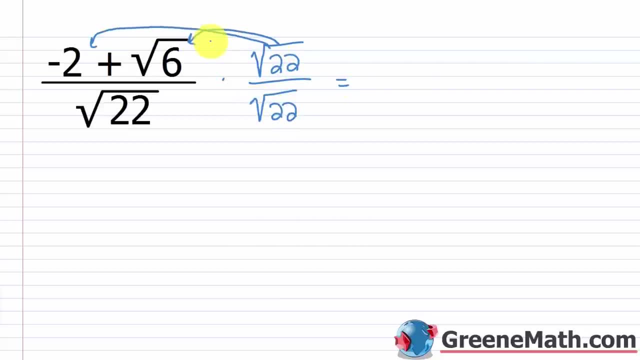 And remember I'm going to multiply the denominator by the square root of 22. And the denominator by the square root of 22. So I'm going to multiply this by both terms. So my numerator becomes what? 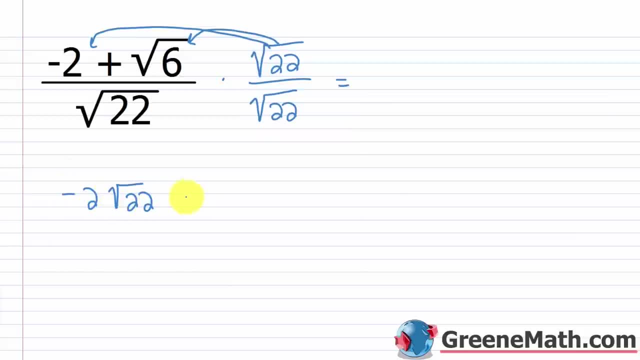 Negative 2 times the square root of 22. Plus we'll have square root of 6 times square root of 22. That'll be the square root of 132. And of course we can simplify that and we'll do that in a minute. 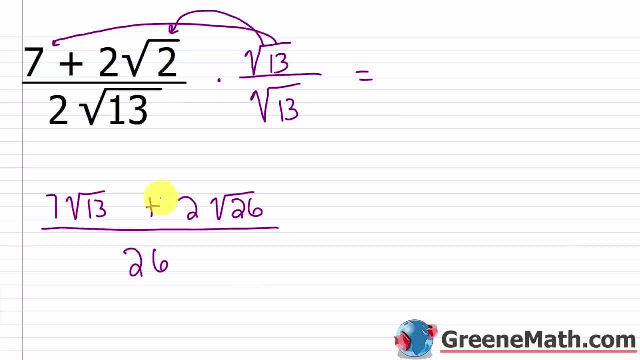 because, remember, we can't just go through and cancel stuff. We've got addition. The biggest mistake students make in Algebra 1 is they start going through and saying, oh, I can cancel this with this, This is 13 now. 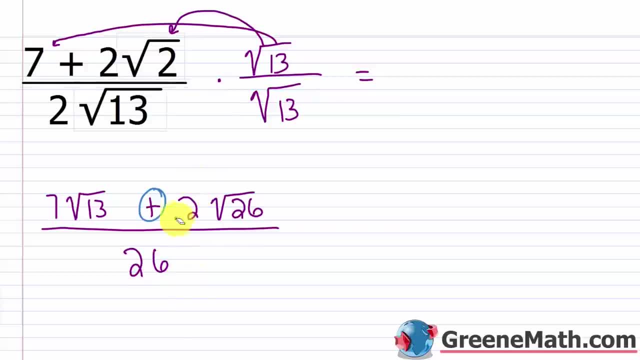 No, you can't do that. Remember: you cancel common factors. So in order for me to be able to cancel this with something up here, I would have to factor something out for it to cancel, And there's nothing that's common that I'm going to be able to factor out. 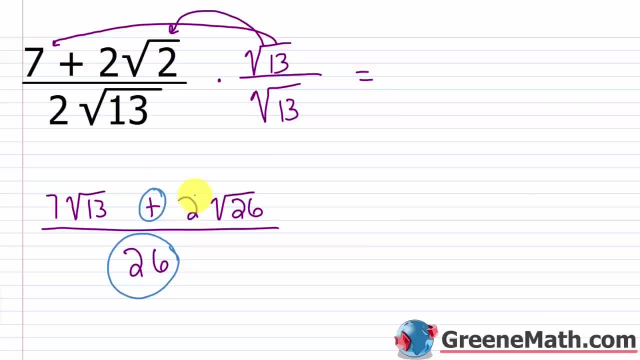 I can't factor out a 2.. This is a 7. This is a 2.. So there's not really anything I'm going to be able to do to simplify this further. I just report my answer at this point and say I have 7 times the square root of 13. 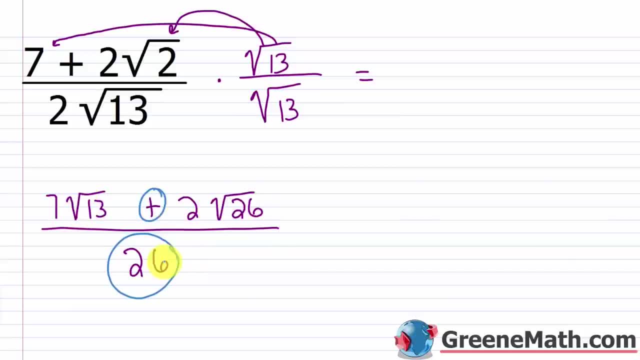 plus 2 times the square root of 26,, and this is over 26.. What about if we come across negative 2 plus the square root of 6, and this is over the square root of 22?? Again, if I look at my problem and I don't see anywhere where I need to. 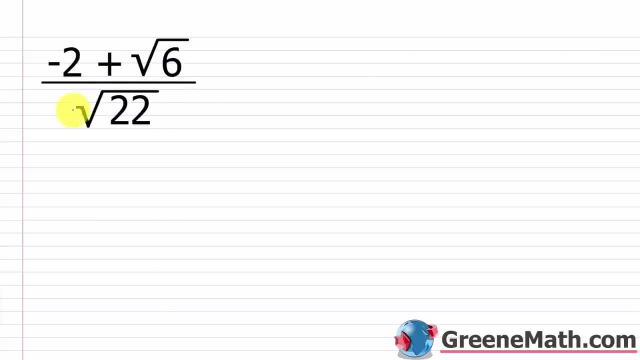 simplify, right. Nothing can be simplified at this point. Well, I'm just thinking about rationalizing the denominator. So I have the square root of 22 down there. So I'm going to multiply the numerator by the square root of 22. 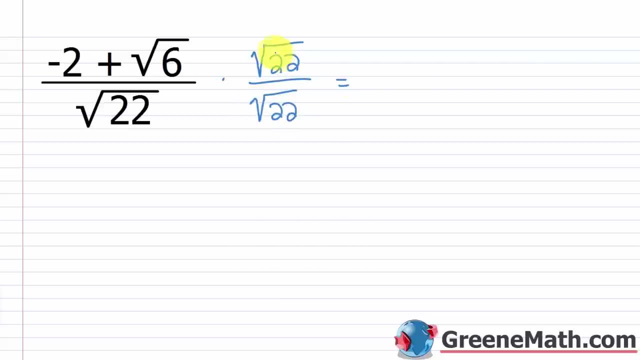 and the denominator by the square root of 22.. And remember, I'm going to multiply this by both terms, So my numerator becomes what Negative 2 times the square root of 22, plus we'll have square root of 6 times square root of 22.. 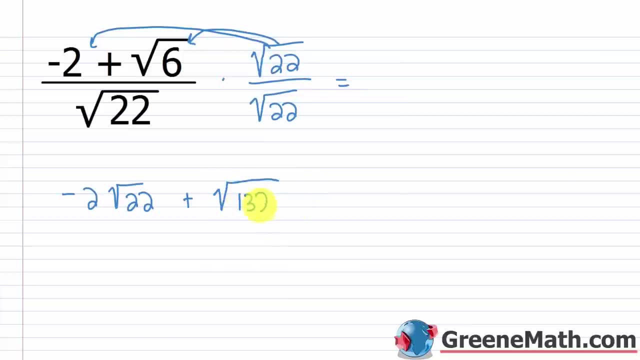 That'll be the square root of 132.. And of course, we can simplify that And we'll do that. We'll do that in a minute, And then this is over. We have the square root of 22 times the square root of 22.. 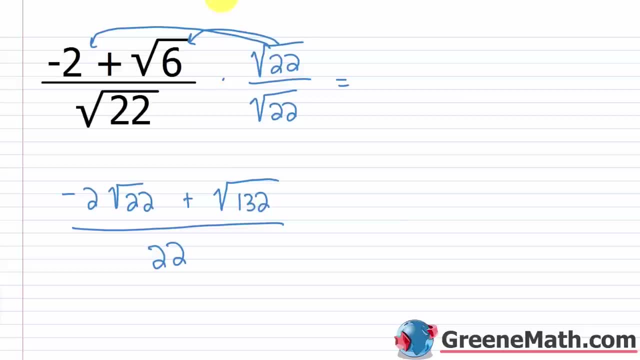 That's going to give me 22.. Now this right here, you should know, can be simplified. I can't do anything with this one, because 22 is what It's 11 times 2.. So there's no perfect square as a factor of 22.. 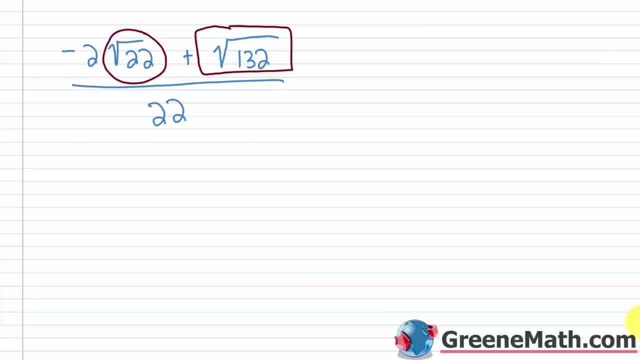 But for 132, a lot of you know 132 is 12 times 11.. So if I have 132 and that's 12 times 11. 12 is what It's 4 times 3.. So 4 is a perfect square. 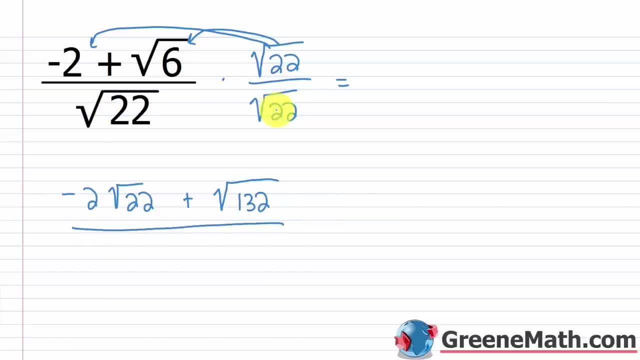 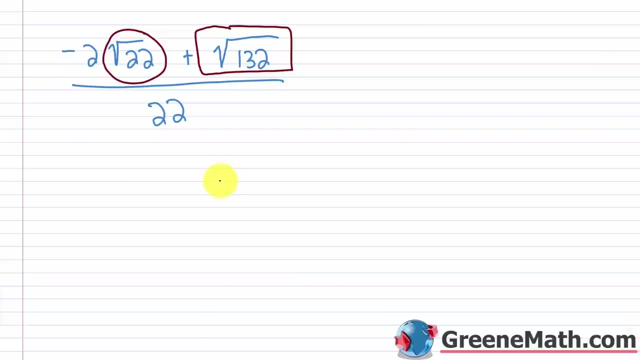 And then this is over. We have the square root of 22 times the square root of 22. That's going to give me 22. Now this right here you should know can be simplified. I can't do this one because 22 is what? It's 11 times 2. So there's no perfect square as a factor of 22. But for 132 a lot of you know 132 is 12 times 11. So if I have 132 and that's 12 times 11. 12 is what? It's 4 times 3. So 4 is a perfect square. So I could really write this as 4 times 33. So let's go ahead and do that. So let's say this is equal to negative 2 times the square root of 22. And then I'm going to put the square root of 33 times the square root of 4 over 22. Okay so now this equals I've got negative 2 times the square root of 22. Plus I know the square root of 4 is 2. So I'm going to put 2 times the square root of 33 over 22. Now is there anything I can do to cancel further? Yes 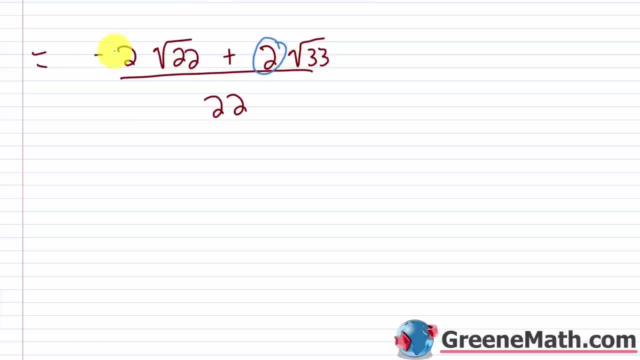 there is. Because in this case I have a 2 here and I have a negative 2 here. But I also can think about that as negative 1 times 2. So if I was to factor a 2 out. Okay from each term in that numerator. So in other words if I said I have 2 and then inside the parentheses I'd have that negative is still there. So negative square root of 22. And then plus factor the 2 out from there. 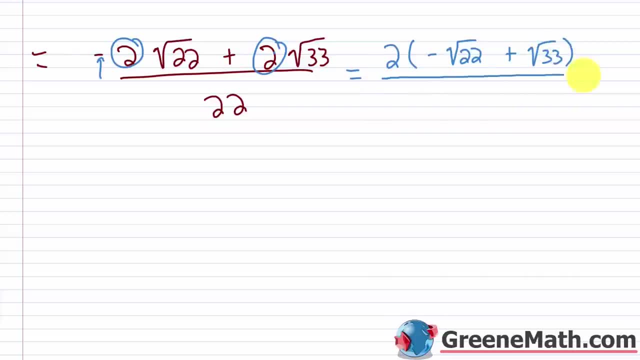 So just square root of 33. And this is over. 22. Now this is multiplication here. 2 is a factor. And this whole thing inside the parentheses here. Negative square root of 22 plus square root of 33 is a factor. So now I can cancel common factors. So this can cancel with a factor of 2 down here. And so this is 11. Okay very important that you understand the difference between when you can cancel and when you can't. Again that's a very very common mistake in Algebra 1. So then this equals. 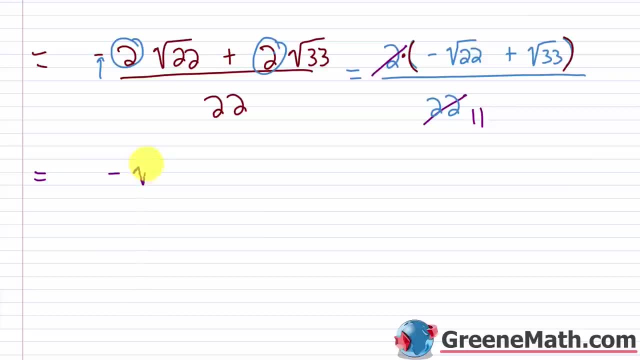 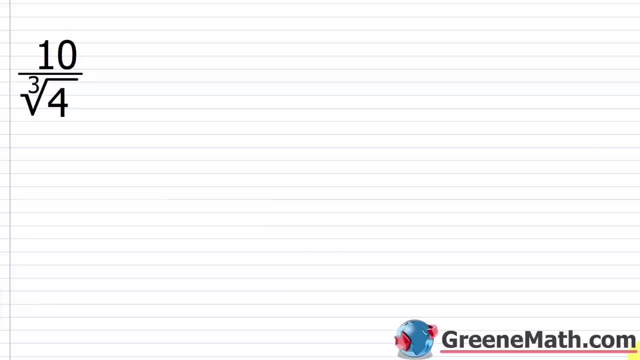 What's left in the numerator after I cancel is a negative square root of 22 plus square root of 33 over 11. Alright so let's take a look at a few now with some higher roots involved. 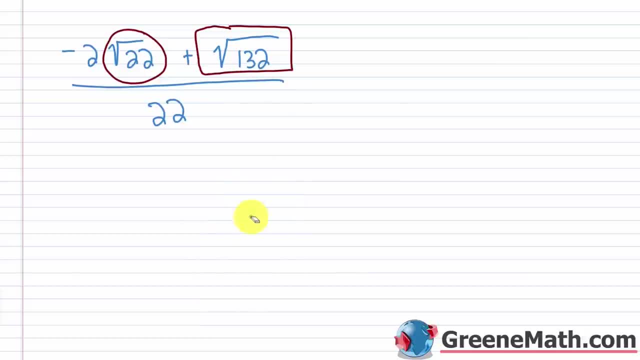 So I could really write this as 4 times 33.. So let's go ahead and do that. So let's say: this is equal to negative, 2 times the square root of 22 plus 33 times 4.. So I'll put the square root of 33 times the square root of 4 over 22.. 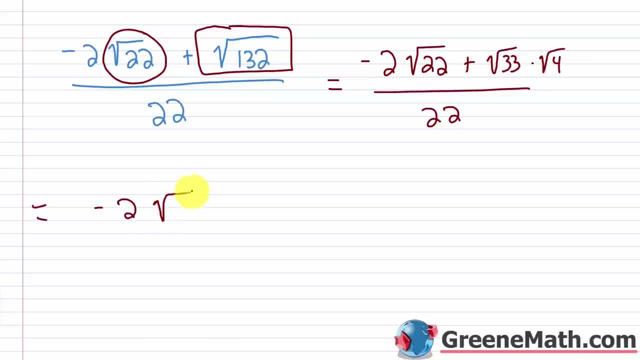 Okay. So now this equals- I've got negative 2 times the square root of 22.. Plus, I know the square root of 4 is 2.. So I'm going to put 2 times the square root of 33 over 22.. 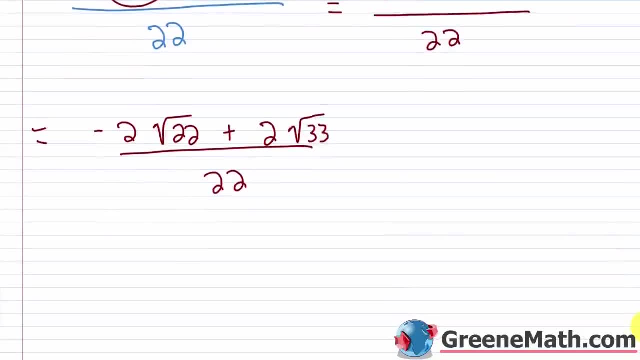 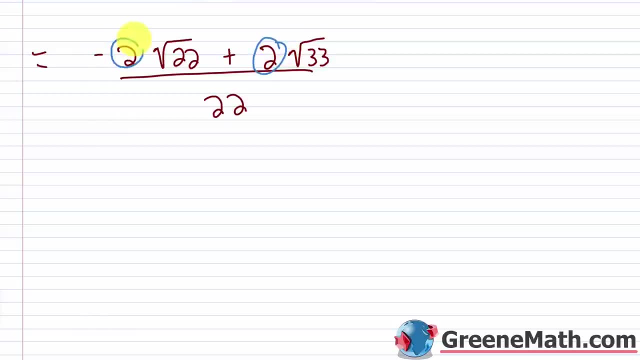 Now, is there anything I can do to cancel further? Yes, there is, Because in this case I have a 2 here and I have a negative 2 here, But I also can think about that as negative 1 times 2.. 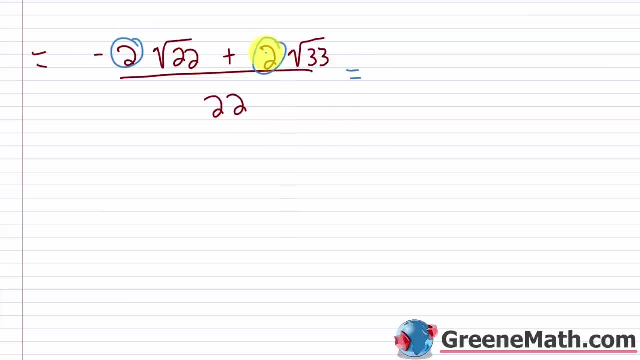 So if I was to factor a 2 out, okay, from each term in that numerator, So in other words, if I said I have 2. And then inside, Inside the parentheses, I'd have that negative is still there. So negative square root of 22.. 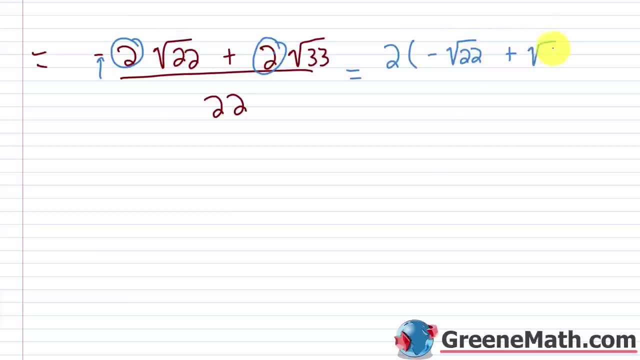 And then plus factor the 2 out from there, So just square root of 33.. And this is over 22.. Now this is multiplication. here 2 is a factor And this whole thing, inside the parentheses here negative. square root of 22 plus square root of 33 is a factor. 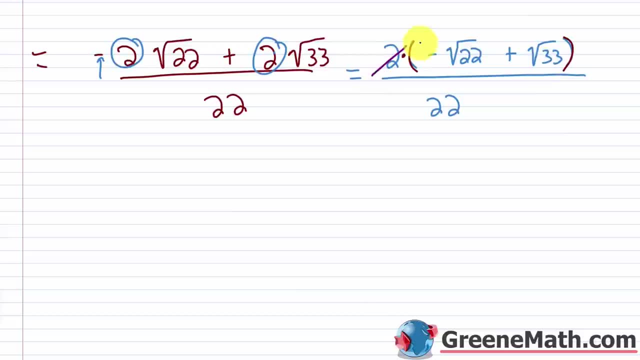 So now I can cancel common factors, So this can cancel with a factor of 2.. So I have a 2 down here, And so this is 11.. Okay, Very important that you understand the difference between when you can cancel and when you can't. 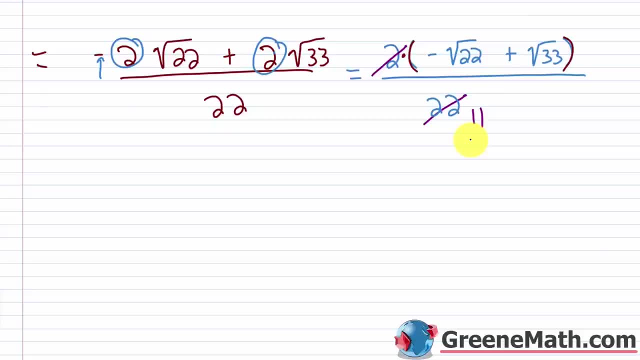 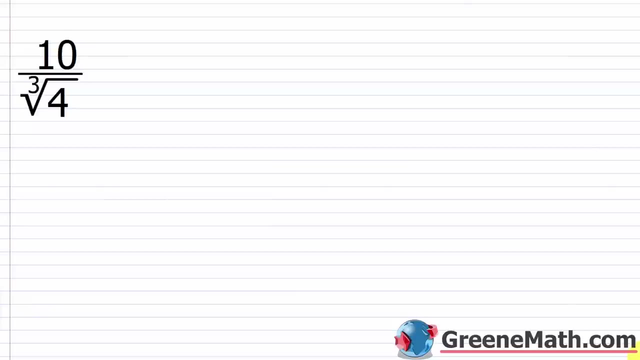 Again, that's a very, very common mistake in Algebra 1.. So then this equals: What's left in the numerator after I cancel is a negative square root of 22 plus square root of 33 over 11.. All right, So let's take a look at a few now with some higher roots involved. 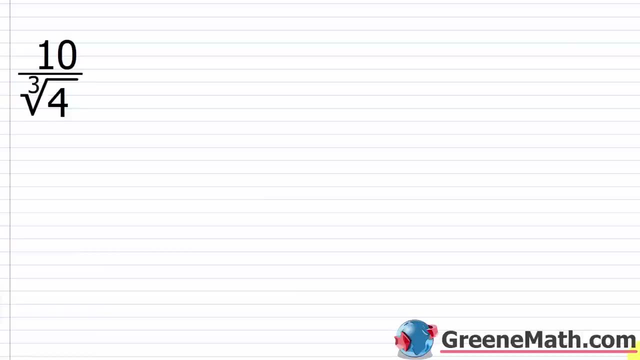 Not much more difficult, Just a little bit more thinking involved. So if I have something like 10 over the cube root of 4, what do I do? A lot of people just come through and they go: okay, well, I'm going to do cube root. 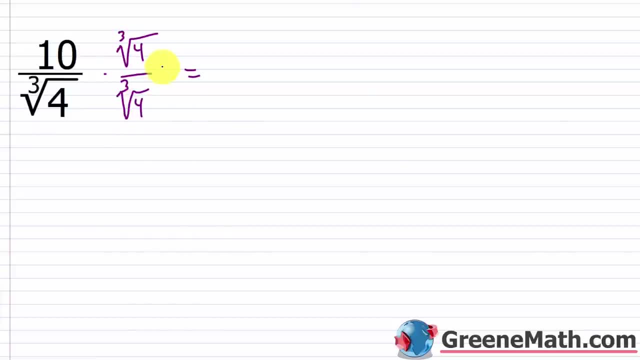 of 4 over cube root of 4.. And okay, 10 times cube root of 4 over 4 times 4 is 16.. So this would be the cube root, the cube root of 16.. Now here's the problem with doing that, particularly when you're getting the higher roots. 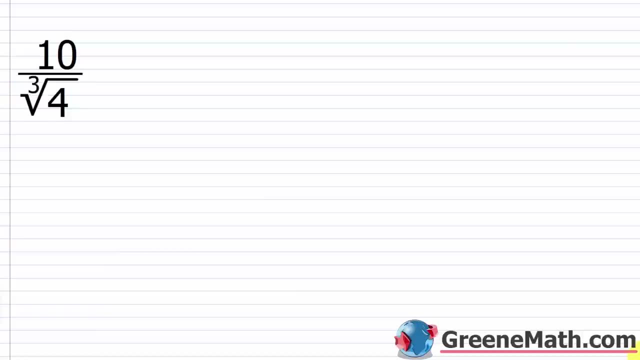 Not much more difficult. Just a little bit more thinking involved. So if I have something like 10 over the cube root of 4. What do I do? A lot of people just come through and they go okay well I'm going to do cube root of 4 over cube root of 4. 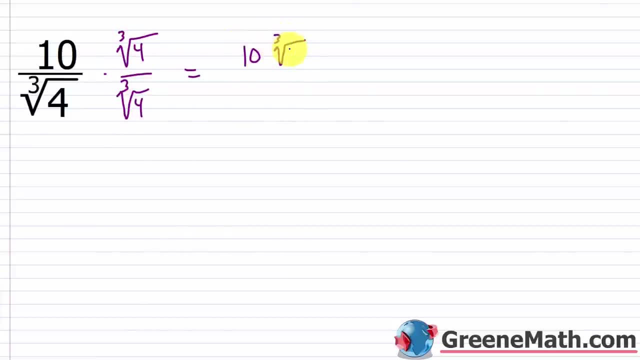 And okay 10 times cube root of 4 over 4 times 4 is 16. So this would be the cube root. The cube root of 16. Now here's the problem with doing that. Particularly when you get into higher roots. This is not simplified. The cube root of 16. 16 is not a perfect cube. This gets broken up into what? The cube root of 8 times the cube root of 2. So this would be 2 times the cube root of 2. of 2 I'd still have a radical in the denominator so this is wrong this is wrong okay what you need to think about here is what do I need to do to get to a perfect cube so in other words if I have 4 here and 4 is 2 squared well I need another 2 another 2 to get to a perfect cube so what I want to multiply by here in this case is the cube root of 2 over the cube root of 2 and what's going to happen is I'm going to have 10 times the cube root of 2 in my numerator over 4 times 2 is 8 so this would be the cube root of 8, 8 is a perfect cube so I would get 10 times the cube root of 2 plus over cube root of 8 is 2. And then I can simplify by canceling a common factor 2 between here and here. So this is a 5. So my final answer there would be 5 times the cube root of 2. Now, another thing you could have done, and I don't advise this, but a lot of students will end up doing this, you could have just taken your opening scenario and done it twice. So in other words, I can say, 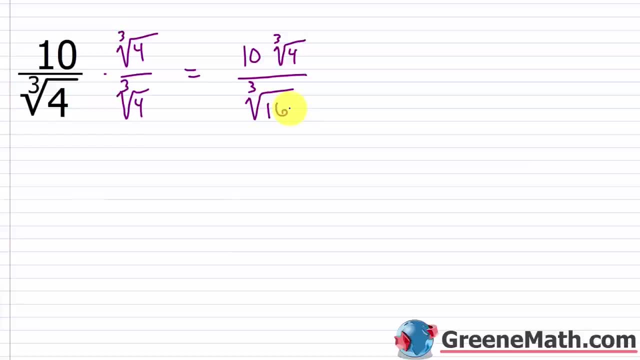 This is not simplified. The cube root of 16,- 16 is not a perfect cube. This gets broken up into what The cube root of 8 times the cube root of 2.. So this would be 2 times the cube root of 2.. 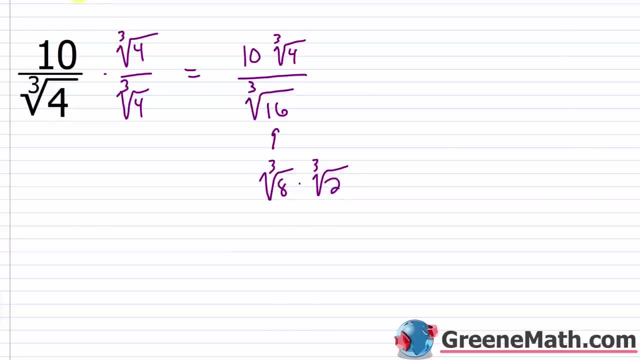 I'd still have a radical in the denominator. So this is wrong. This is wrong. Okay, What you need to think about here is: what do I need to do to get to a perfect cube? So, In other words, if I have 4 here and 4 is 2 squared, well, I need another, 2, another. 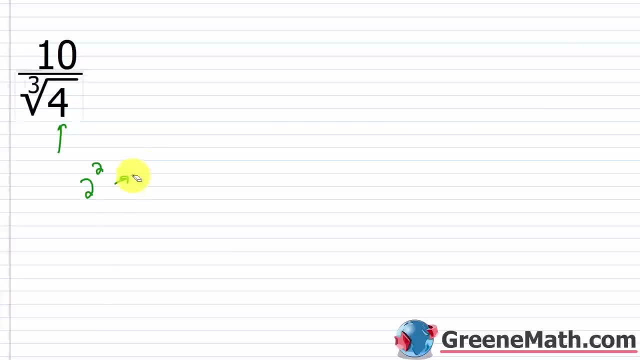 2 to get to a perfect cube. So what I want to multiply by here in this case is the cube root of 2 over the cube root of 2.. And what's going to happen is I'm going to have 10 times the cube root of 2 in my numerator. 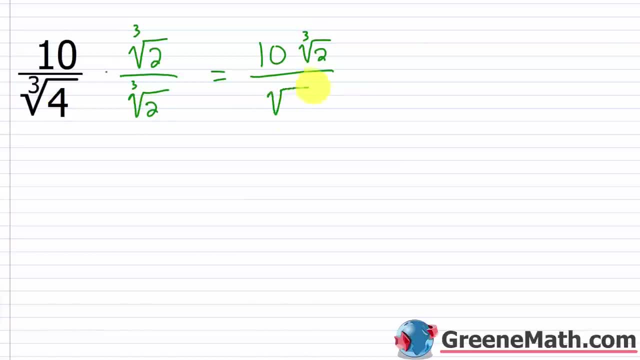 over 4 times 2 is 16.. So this would be the cube root of 8,. 8 is a perfect cube, So I would get 10 times the cube root of 2 over cube root of 8 is 2.. 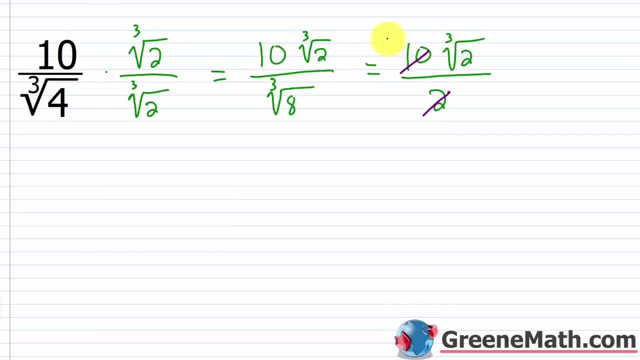 And then I can simplify by canceling the common factor 2 between here and here. So this is a 5.. So my final answer: there would be 5 times the cube root of 2.. Now another thing you could have done, and I don't advise this, but a lot of students 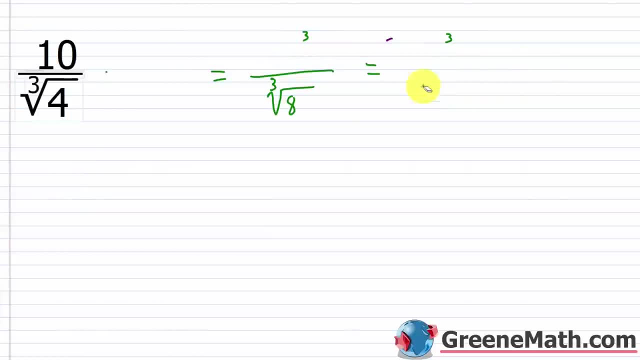 will end up doing this. You could have just taken your opening scenario and done it twice. So in other words, I can say: well, I've got cube root of 4 there, so I can just multiply this by cube root of 4 times cube root of 4.. 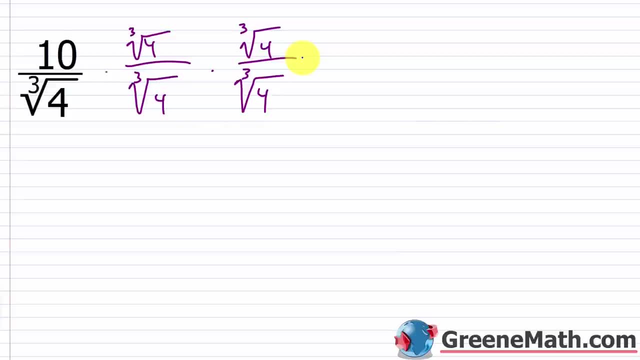 And I see a lot of students doing this and I don't know why you wouldn't just do the couple extra seconds to get the, you know, easier calculation. But if you want to do this, you can. It's going to give you the right answer. it's just a little bit more work. 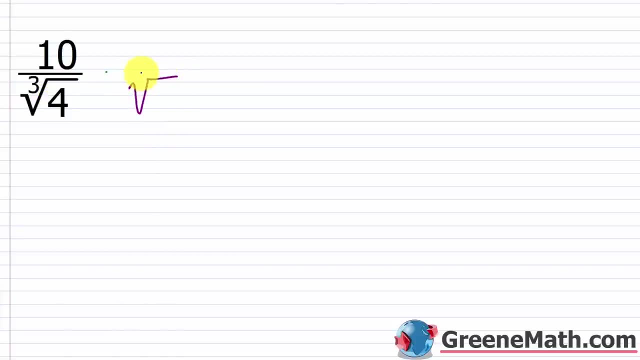 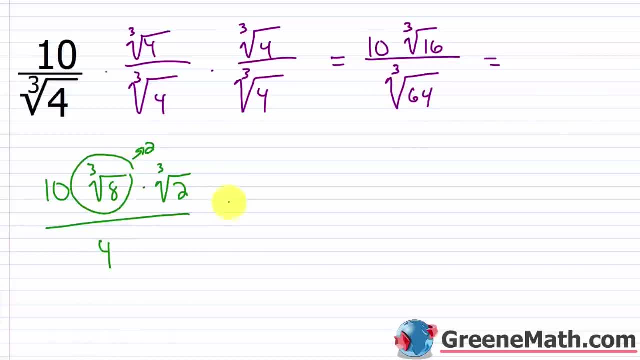 The cube root of 64 is 4. So let's write that as 4. Okay, so now I have 2 times 10, which is 20 times the cube root of 2 over 4. So now I've done all that extra work. And I'm going to get the same answer. 20 divided by 4 is 5. So either way, I'm going to end up with what? 5 times the cube root of 2. So again, if you want to do this, you can. But it's going to just take you longer to get the 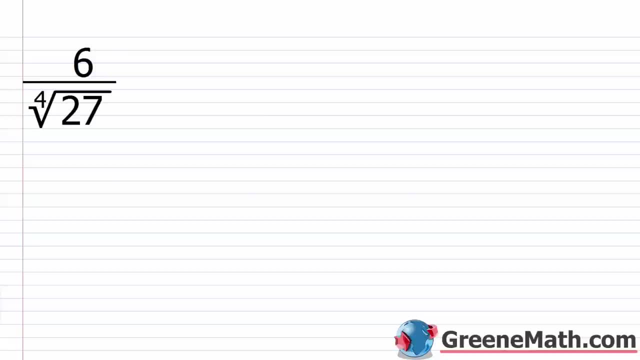 final simplified answer. So I'm going to write that as 4. So I'm going to write that as 4. So let me just say this as a rule. I would like for you, as a student, to try to get in the habit of 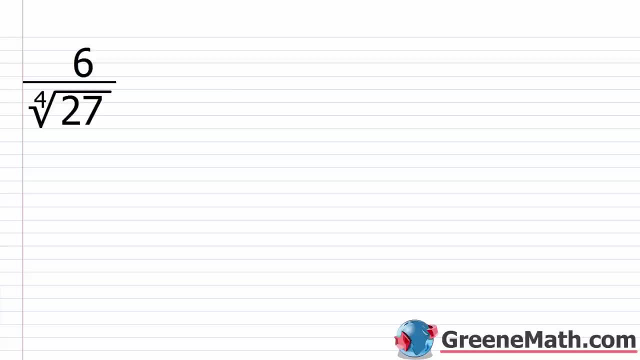 multiplying by the smallest radical possible, because this is going to cut down on the amount of simplification you have to do. That's what you always want to think about. How can I multiply by the smallest radical possible? So let's take a look at one final problem. And I want you to just 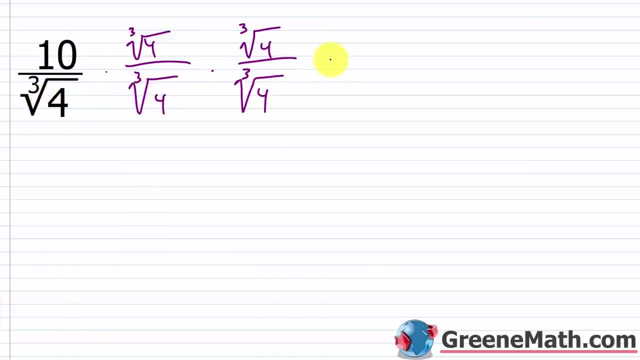 So if I multiply The cube root of 4 times the cube root of 4 times the cube root of 4, I would end up with what? The cube root of 64. That's my denominator, And then in the numerator I would have 10 times the cube root of 16.. 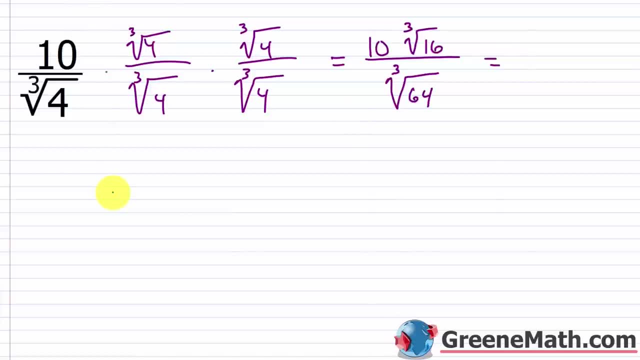 Now a lot more work. to simplify, when you do this, The cube root of 16 is the cube root of 8 times the cube root of 2.. So let me write 10 times the cube root of 8 times the cube root of 16.. 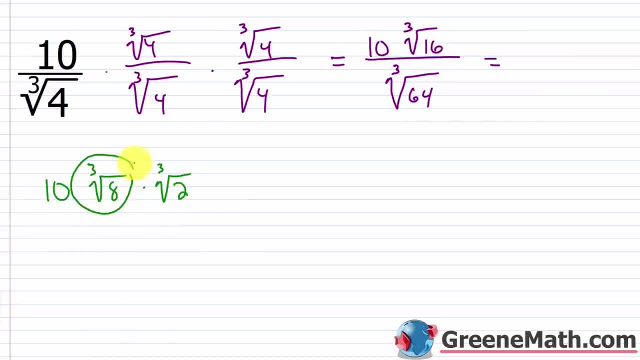 That's my denominator. Now we know this is 2, so we'll simplify that in a minute. The cube root of 64 is 4.. Let's write that as 4.. Okay, So now I have 2 times 10,, which is 20, times the cube root of 2 over 4.. 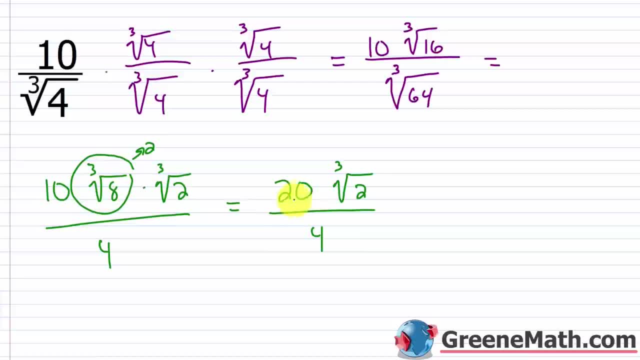 So now I've done all that extra work and I'm going to get the same answer: 20 divided by 4 is 5.. So either way, I'm going to end up with what? 5 times the cube root of 2.. 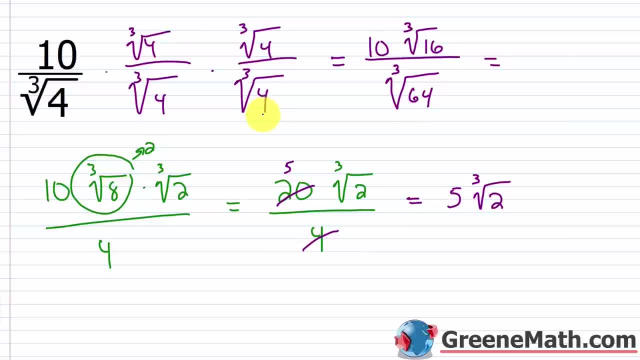 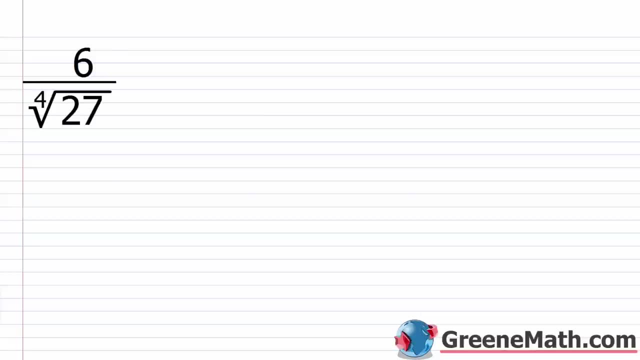 So if you want to do this, you can, but it's going to just take you longer to get the final simplified result in the end. so let me just say this as a rule: i would like for you, as a student, to try to get in the habit of multiplying by the smallest radical possible, because this is going to cut down. 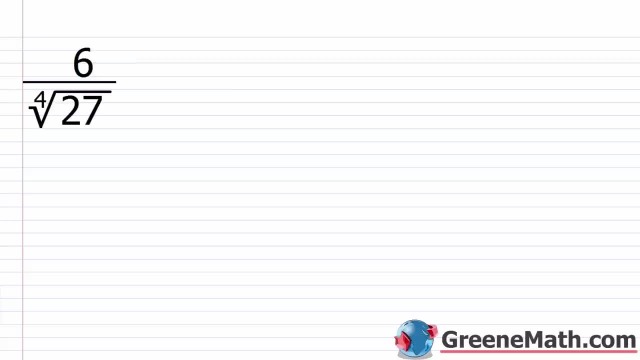 on the amount of simplification you have to do. that's what you always want to think about: how can i multiply by the smallest radical possible? so let's take a look at one final problem, and i want you to just think about it. just pause the video and think about what's the 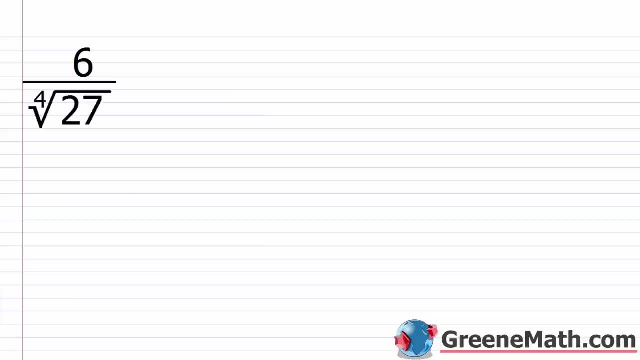 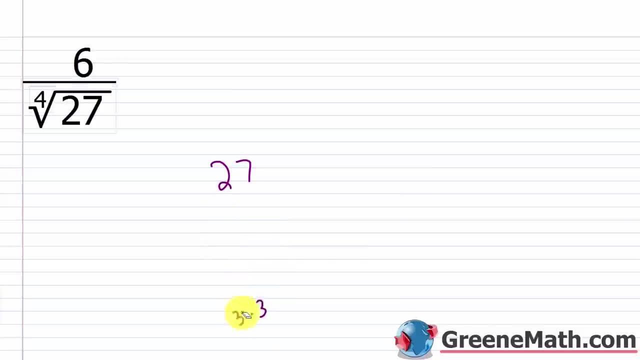 cubed. now, if it's three cubed, if it's three cubed and i have an index of four, what does that tell you? i need to multiply by one more three. three cubed times three to the first power will give me three to the fourth power. so that's a perfect fourth right. three to the fourth power is 81. that's what. 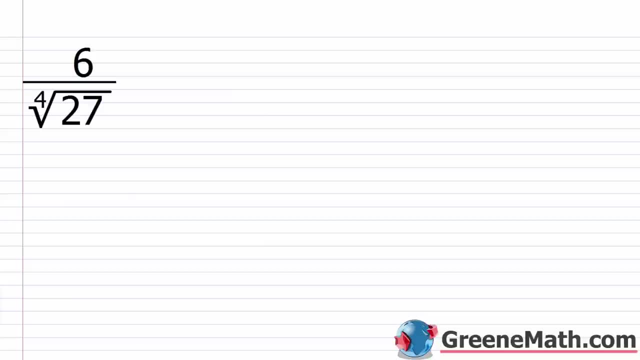 think about it. Just pause the video and think about what's the smallest radical possible? What's the smallest radical I can multiply by to accomplish this? All right. So if you've tried this, you would see, OK, you have 6 over the fourth root of 27. What is 27? Just start with that. Well, it's what? It's 9 times 3. And then 9 is 3 times 3. So really, it's 3 cubed. Now, if it's 3 cubed, if it's 3 cubed, and I have an index of 4, what does that tell you I need to multiply by? 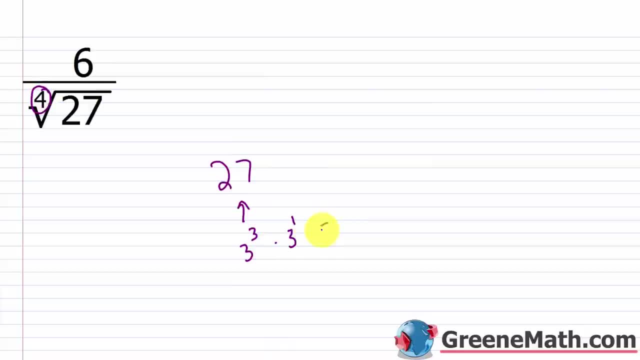 One more 3. 3 cubed times 3 to the first power will give me 3 to the fourth power. So that's a perfect fourth, right? 3 to the fourth power is 81. That's what we'd be looking for here as the smallest radical, which would be the fourth root of 3, to multiply by to simplify this thing. So I want to multiply the numerator by the fourth root of 3 and the denominator by the fourth root of 3. And this will equal what? And the numerator, just 6 times the fourth root of 3. And the denominator, the fourth root of 27 times the fourth root of 3 is the fourth root of 81. And I know the fourth root of 81 is 3. So this equals 6 times the fourth root of 3 over, again, this is 3. Now, I can cancel here 6 and 3. 6 divided by 3 is 2. So this would be 2. And I end up with what? 2 times the fourth root of 3. And I end up with 4 times the fourth root of 3. Now, again, if you wanted to do this, a lot of students will look at that right there and say, oh, what am I going to do? So they'll multiply by the fourth root of 27 4 times, okay? Please don't do stuff like that. It's just, it's way too much work. It's too complicated. Take 5 seconds and build a factor tree and figure out what is the smallest radical that I can multiply by to accomplish this goal. That's what I'm going to do. 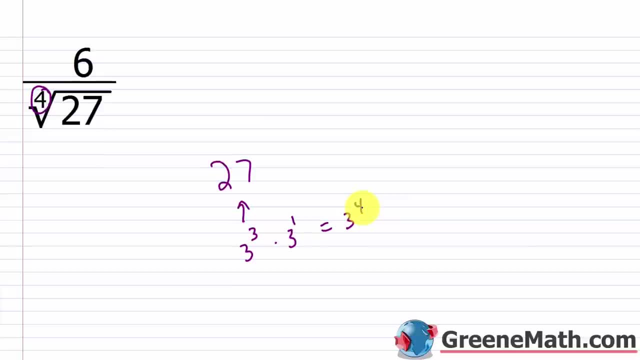 we'd be looking for here as the smallest radical, which would be the fourth root of three, to multiply by what's the smallest radical, which would be the fourth root of three. to multiply by three, корface by, to simplify this thing. So I want to multiply the numerator by the fourth root of three. 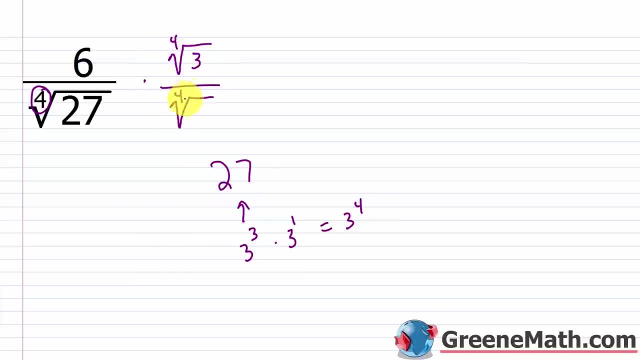 and the denominator by the fourth root of three, and this will equal what In the numerator, just six times the fourth root of three. In the denominator, the fourth root of 27 times the fourth root of three, is the fourth root of 81. And I know the fourth root of 81 is three. so this: 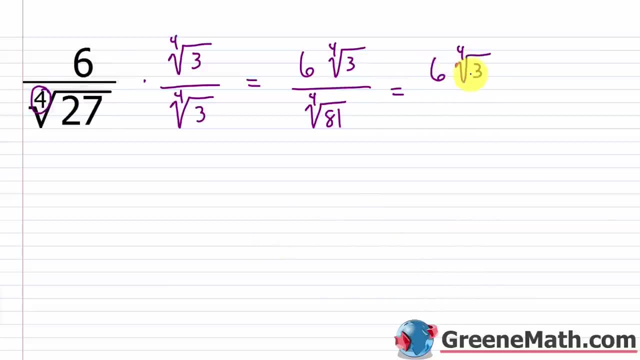 equals six times the fourth root of three. over again, this is three. Now I can cancel here six and three. Six divided by three is two, So this would be two, and I end up with what? Two times the fourth root of three. Now again, if you wanted to do this, a lot of students will look at that. 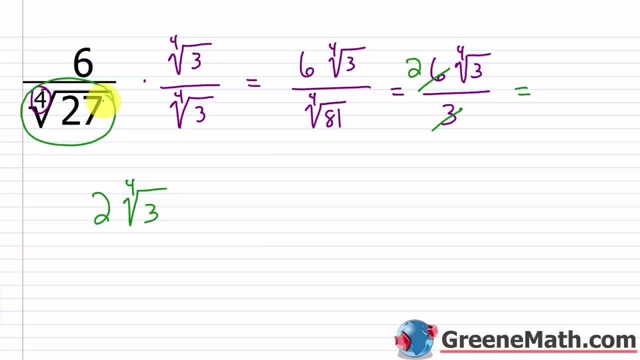 right there and say, oh, what am I going to do? So they'll multiply by the fourth root of 27 four times. Okay, please don't do stuff like that. It's just, it's way too much work, It's too complicated. Take five seconds and build a factor tree and figure out what is the smallest radical. 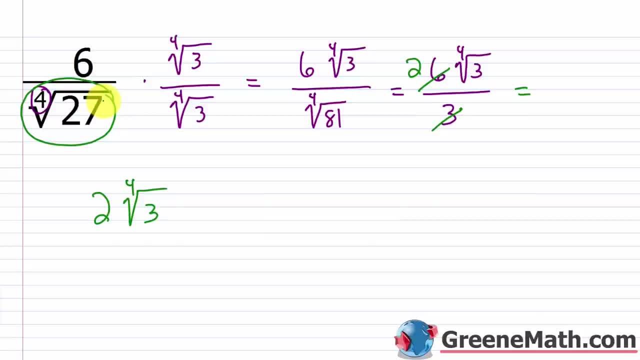 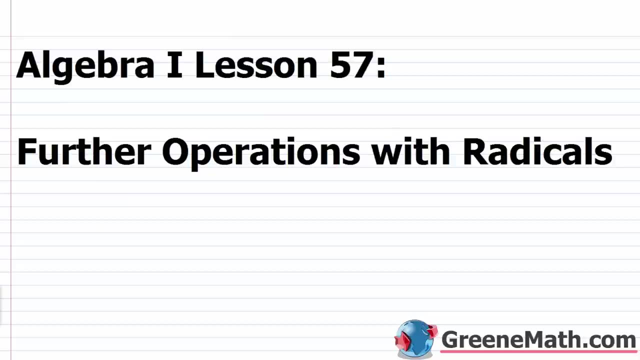 that I can multiply by to accomplish this goal. That's going to save you so much work in the end. Hello and welcome to Algebra 1, Lesson 57. In this video, we're going to learn about further operations with radicals. So before I begin this lesson, I want to revisit. 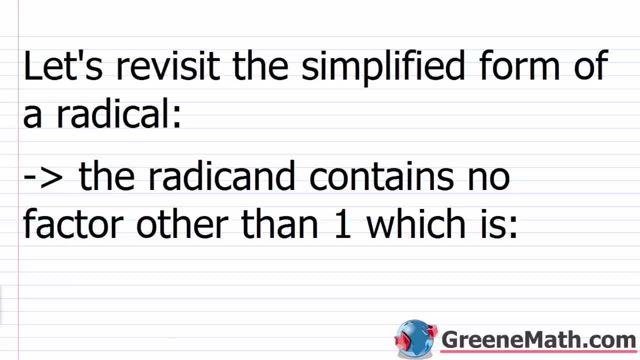 the simplified algebra. So what is a simplified form of a radical that we learned in the last section, So kind of? the first rule that we encountered was that the radicand- remember that's your number or your variable, or your expression- that's under the radical symbol. Okay, so this contains no factor other than one. 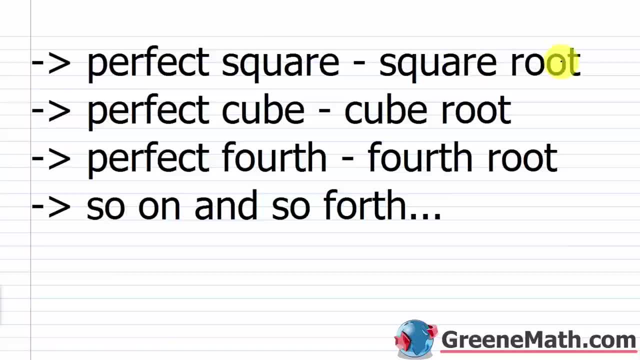 which is: and then we have a perfect square in the case of a square root, a perfect cube in the case of a cube root, a perfect fourth in the case of a fourth root, and then so on and so forth. So, as an example of this, I typically use the square root of 8.. So if I have something like the 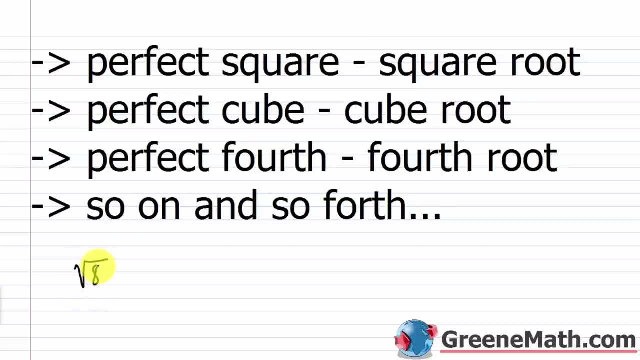 square root of 8.. At this point in algebra, we all know that 8 is 4 times 2.. And we should know that 4 is a perfect square: It consists of 2 times 2.. So this is not considered simplified because 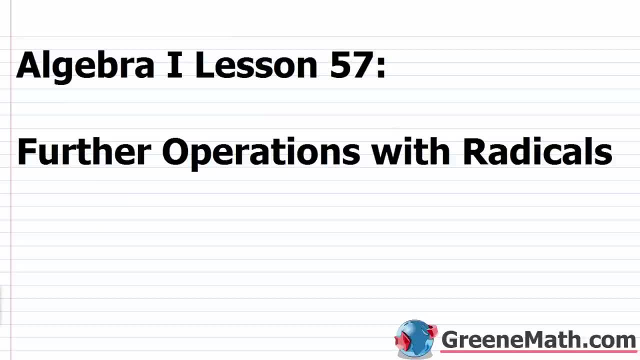 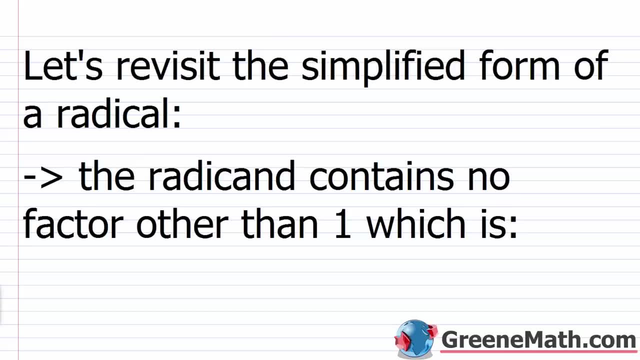 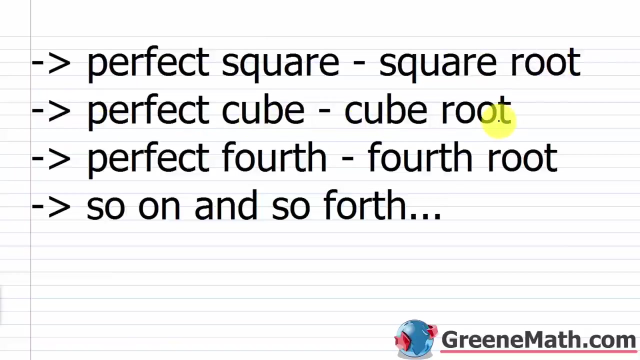 It's going to save you so much work in the end. Hello, and welcome to Algebra 1 Lesson 57. In this video, we're going to learn about further operations with radicals. So before I begin this lesson, I want to revisit the simplified form of a radical that we learned in the last section. So kind of the first rule that we encountered was that the radicand, remember, that's your number or your variable or your expression that's under the radical symbol. Okay, so this contains no factor other than 1, which is, and then we have a perfect square in the case of a square root, a perfect cube in the case of a cube root, a perfect fourth in the case of a fourth root, and then so on and so forth. So as an example of this, I typically use the square root of 8. So if I have something like the square root of 8. At this point in algebra, we all know that 8 is 4 times 2. And we should know that 4 is a perfect square, right? It consists of 2 times 2. So this is a perfect square. So I can put that this is equal to, and I can split this up as the square root of 4 times the square root of 2. And I can say that the square root of 4 represents a rational number 2, right? It's a perfect square. So what they want me to do in order to simplify this is just to replace this with a 2, right? Replace it with its rational number. So I'd have to do this. 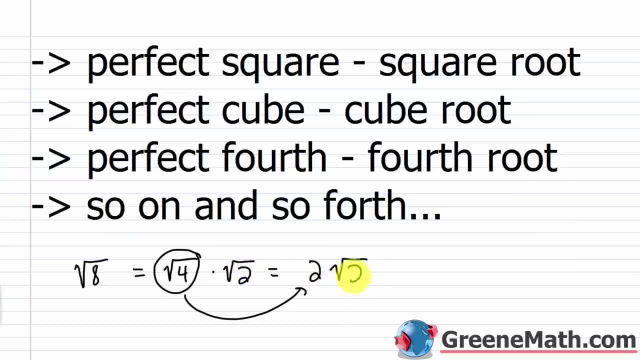 I'd have 2 times the square root of 2, which I can't simplify. So there's no difference between this guy right here, 2 times the square root of 2, and the square root of 8 in terms of its value, right? Punch them both in on a calculator, you get the same thing. But if you turn this in on a test, you're probably not going to get full credit because it's not considered simplified, okay? 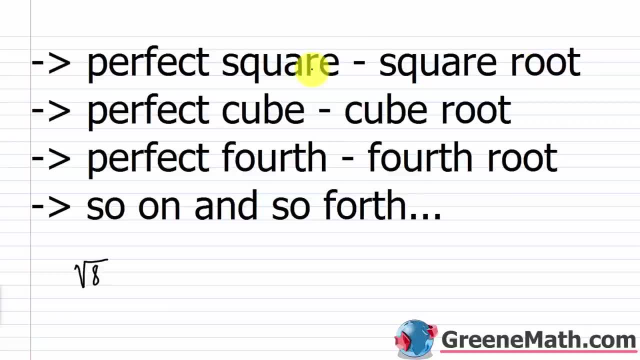 it's a square root and one of its factors is a perfect square, And one of its factors again is 4.. So I can put that this is equal to, and I can split this up as the square root of 4 times the root of two, And I can say that the square root of four represents a rational number two, right. 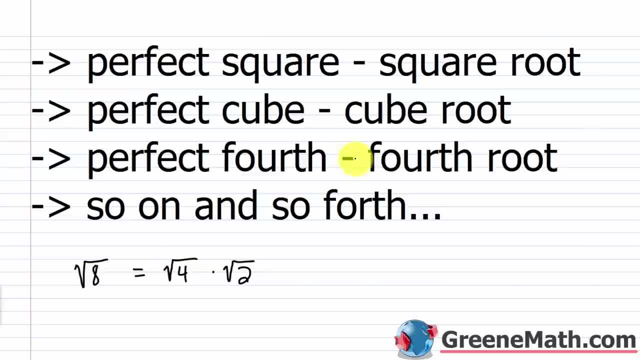 It's a perfect square. So what they want me to do in order to simplify this is just to replace this with a two right, Replace it with its rational number, So I'd have two times the square root of two, which I can't simplify. So there's no difference between this guy right here two times. 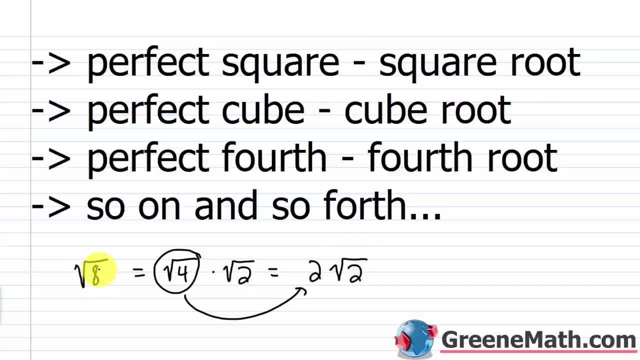 square root of two and the square root of eight in terms of its value right. Punch them both in on a calculator. you get the same thing. But if you turn this in on a test, you're probably not going to get full credit because it's not considered simplified. okay, And let me do an 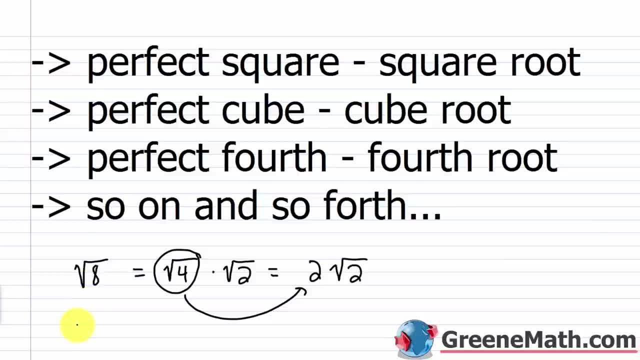 example, with a perfect cube, Let's say we had the cube root of 16,. okay, That's going to keep it nice and simple. I know that this consists of what 16 I could do as eight times two and eight is a. 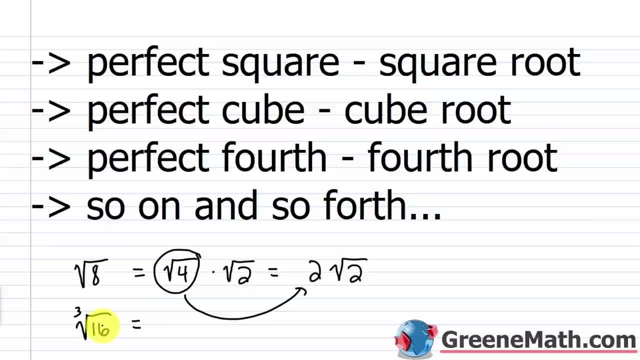 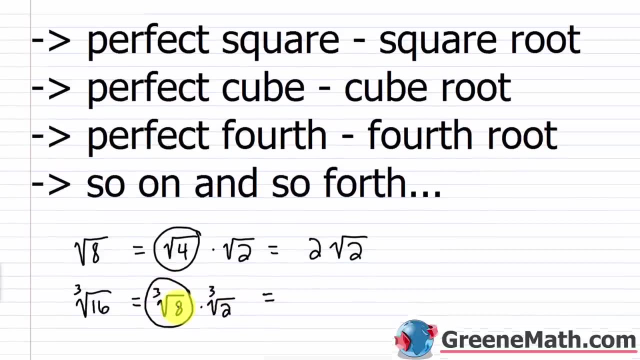 perfect cube. So again, one of the factors of 16 is a perfect cube. So I would break this up and say: this is the cube root of eight times the cube root of two, And again this represents a rational number. The cube root of eight is two. 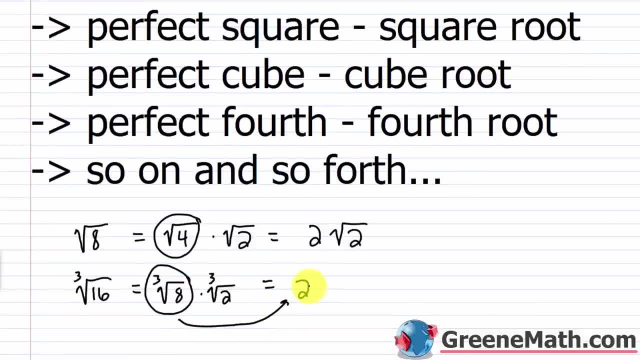 So I'm simply going to write this as two in the simplified version, and then I'm going to keep what doesn't simplify. So times the cube root, the cube root of two. So two times the cube root of two is simplified. The cube root of 16 is just unsimplified Again. 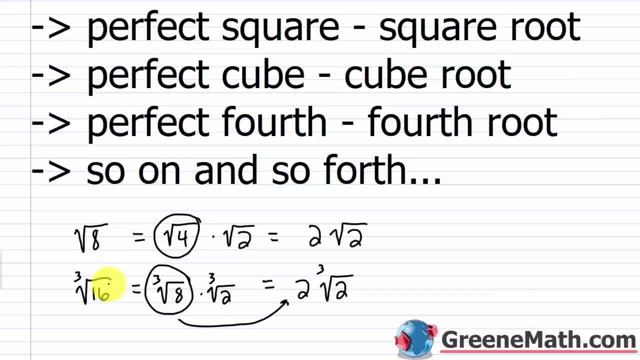 represent the same value. And you could go on and on when you talk about a fourth root and look for a perfect fourth in one of the factors of the radicand right, Or you could do that with a fifth root or sixth root, you know so on and so forth. All right, So kind of the next thing we talked. 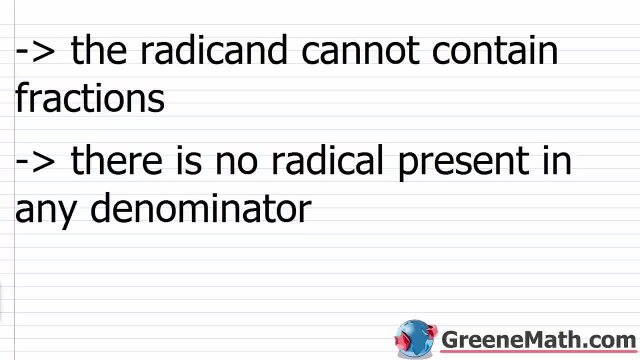 about was that the radicand cannot contain fractions. So if I saw something like, let's say, the square root of two over 25, something like that, this would not be considered simplified. So what they want you to do is break this up using your quotient rule for 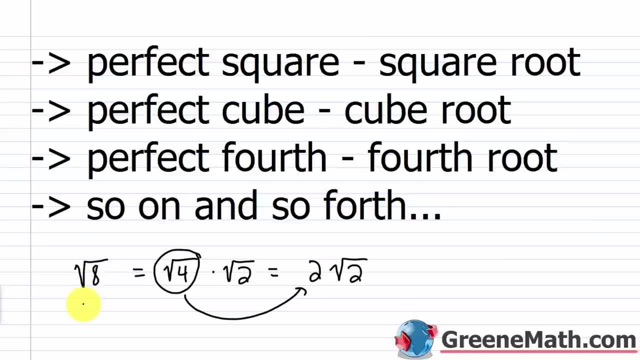 And let me do an example with a perfect cube. Let's say we had the cube root of 16. Okay, that's going to keep it nice and simple. I know that this consists of what? 16 I could do as 8 times 2, and 8 is a perfect cube. So again, one of the factors of 16 is a perfect cube. So I would break this up and say this is the cube root of 8 times the cube root of 2. And again, this represents a rational number. The cube root of 8 is 2. So I'm simply going to write this as 2 in the simplified version. 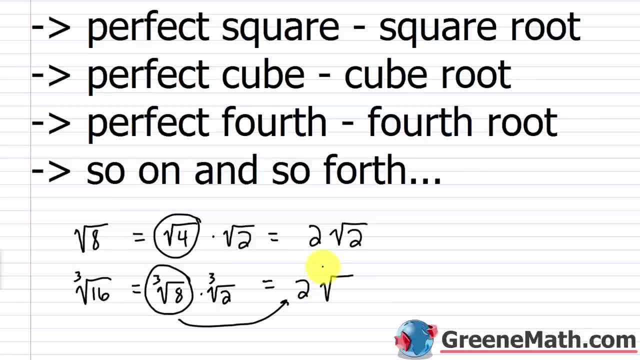 And then I'm going to keep what doesn't simplify. So times the cube root, the cube root of 2. So 2 times the cube root of 2 is simplified. The cube root of 16 is just unsimplified. Again, they represent the same value. And you could go on and on when you talk about a, you know, a fourth root and look for a perfect fourth in one of the factors of the radicand, right? Or you could do that with a fifth root or sixth root, you know, so on and so forth. All right, so kind of the next thing we talked about was the cube root of 8 times the cube root of 2. And I'm going to keep what doesn't 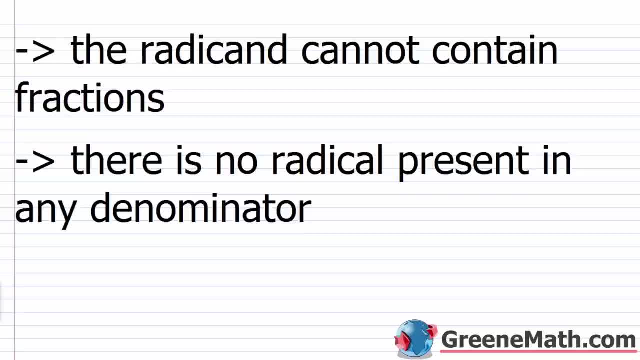 simplify. So what this game came up with was that the radicand cannot contain fractions. So if I saw something like, let's say, the square root of 2 over 25, something like that, this would not be considered simplified. So what they want you to do is break this up using your quotient rule for radicals. So this would be what? The square root of 2 for the numerator over the square root of 25 for the denominator. And the square root of 25 happens to be a radical. So what I want to do is break this up using the quotient rule for radicals. So this would be what? The square root of 2 for the rational number, right? It's 5. So let's just replace that with a 5. So we'd have the square root of 2 over 5. And again, this would just be the simplified version of that. Then kind of the last thing that we talked about was that there is no radical presence in any denominator. So you'll 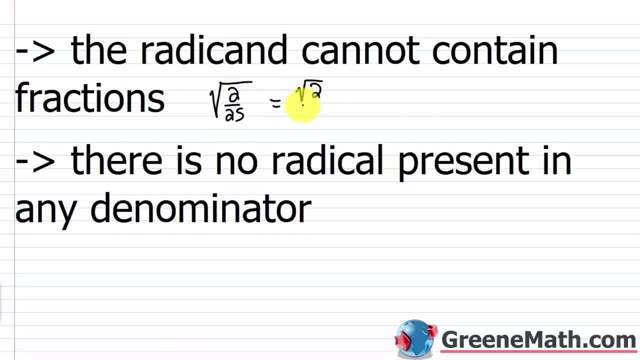 radicals. So this would be what: The square root of two for the numerator over the square root of 25 for the denominator. And the square root of 25 happens to be a rational number. right, It's five. So let's just replace that with a five, So we'd have the square root of two over five, And again. 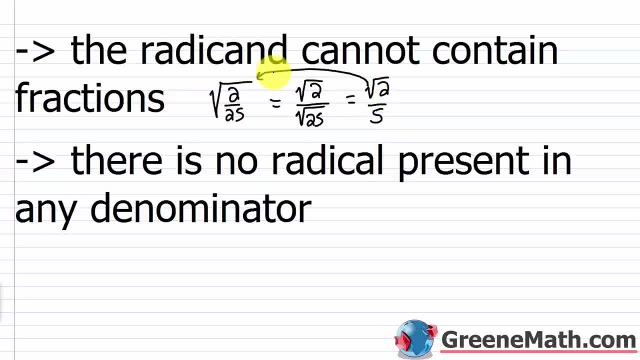 this would just be the simplified version of that. Then, kind of the last thing that we talked about was that there is no radical presence in any denominator. So you'll recall that this was basically the focus of the last section where we learned about rationalizing the denominator. So 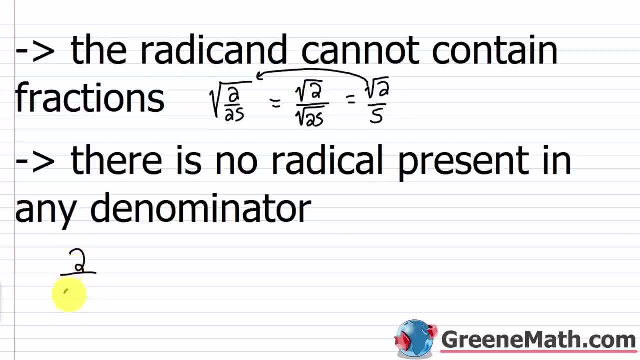 if I had something like two over the square root of seven. we said that this, right here, was an irrational number, right Square root of seven. So we want to rationalize this denominator And in order to do that, I'd multiply both the numerator and denominator by the square root of. 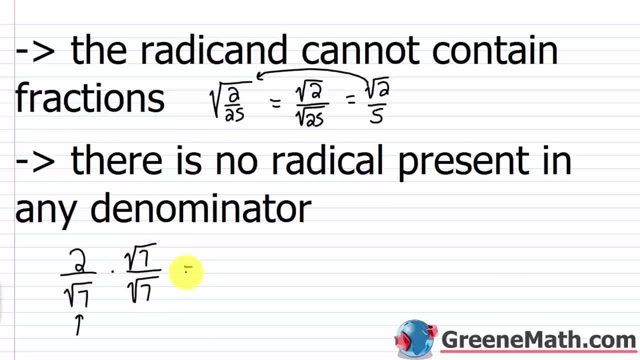 seven, And so square root of seven times square root of seven would be seven. And I went from an irrational number, square root of seven, to a rational number which is seven. So that's where you get rationalizing the denominator from Then in the numerator you just have two times the. 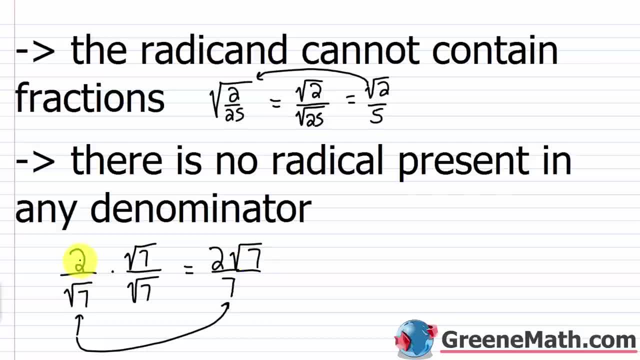 square root of seven. So again, these two: two over the square root of seven and two times square root of seven over seven. they represent the same value. It's just that this one is simplified and this one is not. So if you're going to do this, you're going to have to do this, So you're going to. 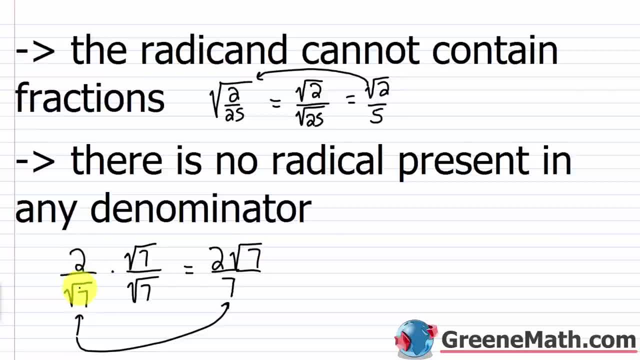 report something like this on your test as an answer. You might get a wrong answer, You might get points taken away. Your teacher might forgive you and give you full credit, But in a lot of scenarios you're going to at least lose some points for not simplifying and reporting your 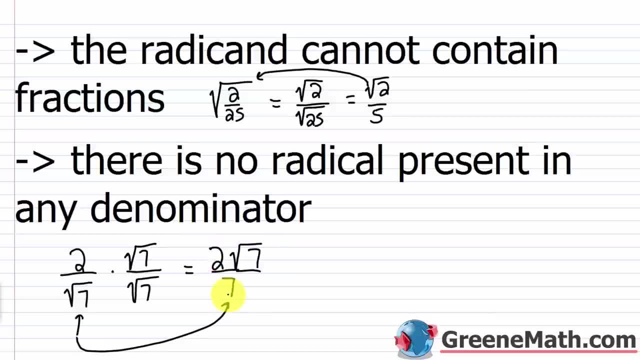 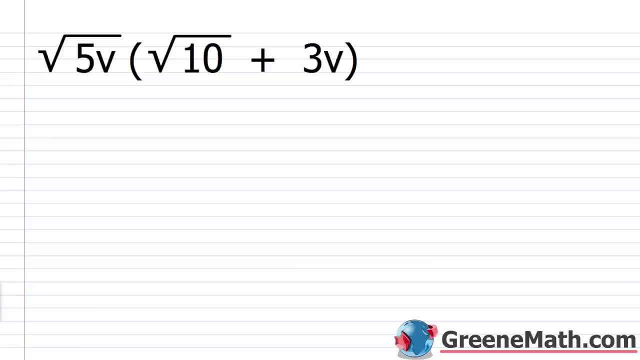 answer in this way. It's just like if you reported a fraction- something like two-fourths- right. You don't want to do that. You want to simplify and say it's one-half. So what we're going to do now is we're going to use all the knowledge we've gained so far. 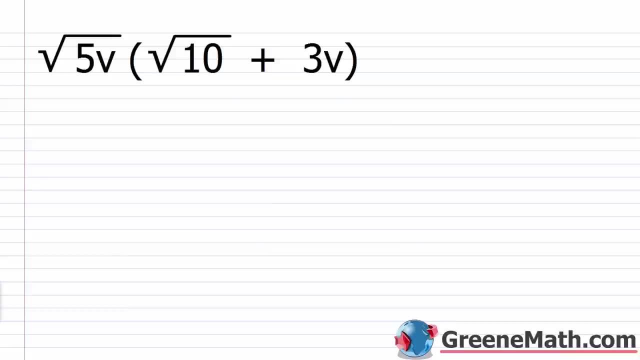 And we're just going to look at some typical problems that you will encounter with radicals. I'm keeping it very simple here for Algebra 1.. When we get to Algebra 2, College Algebra, we're going to look at some very, very difficult problems. So for right now, let's just keep it. 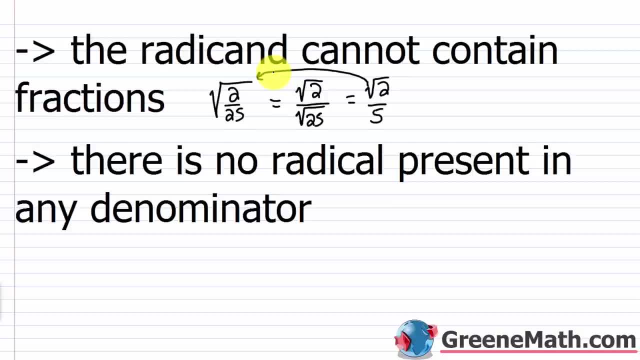 recall that this was basically the focus of the last section where we learned about rationalizing the denominator. So if I had something like 2 over the square root of 7, we said that this right here was an irrational number, right? Square root of 7. So we want to rationalize this denominator. And in order to do that, I'd multiply both the numerator and denominator by the square root of 7. And so square root of 7 times square root of 7 would be 7. And I went from an irrational number, square root of 7, to a rational number, square root of 7, which is 7. So that's where you get rationalizing the denominator from. Then in the numerator, you just have 2 times the square root of 7. So again, these two, 2 over the square root of 7 and 2 times the square root of 7 over 7, they represent the same value. It's just that this one is simplified and this one is not. So if you report something like this on your test as an answer, you might get a wrong answer. You might get points taken away. Your teacher might forgive you and, you know, give you full credit. But in a lot of cases, you might get a wrong answer. 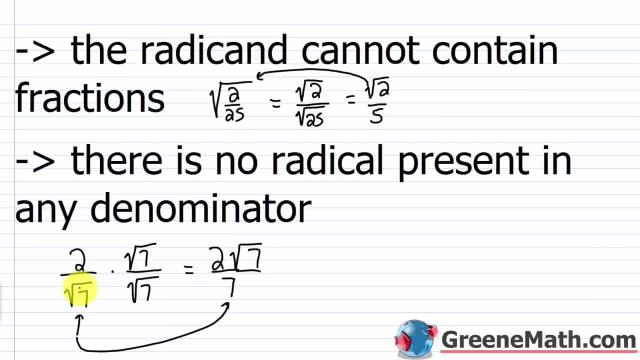 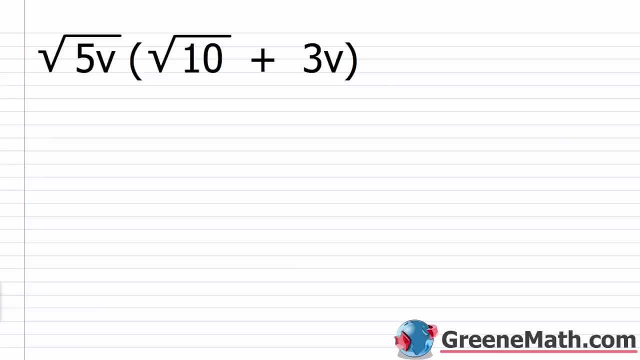 In a lot of scenarios, you're going to at least lose some points for not simplifying and reporting your answer in this way. It's just like if you reported a fraction, something like two-fourths, right? You don't want to do that. You want to simplify and say it's one-half. So what we're going to do now is we're going to use all the knowledge we've gained so far, and we're just going to look at some typical problems that you will encounter with radicals. I'm keeping it very simple here for Algebra 1. When we get to Algebra 2, College Algebra, we're going to look at some very, very difficult problems. So for right now, let's just keep it simple. And let's start out with the square root of 5v times the quantity, the square root of 10 plus 3v. So what I'm going to do here, because these are not able to be combined inside the parentheses here, I'm going to use my distributive property to simplify. So I'm going to multiply this times this and also times this, and we're going to see what we can simplify. So we'll have the square root, the square root of 5v, multiplied by the square root of 10, and then plus the square root of 5v multiplied by 3v. Now, can I do anything to simplify here? Well, yes, I can. The square root of 5v times the square root of 10, I could write that as what? The square root of 5 times 10. Think about breaking this down completely. Square root of 5 times square root of 5 times square root of 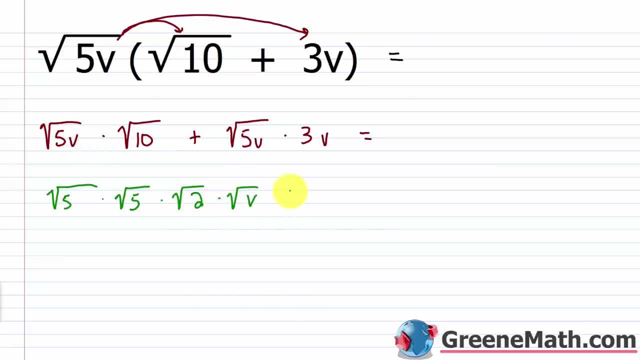 10, and then times square root of v. Then plus. Over here, the square root of 5v, I could break that down, but really I'm not going to be able to do anything with that. 5 is prime, v is to the first power, nothing I can really do. So then times 3v. I can do stuff here because the square root of 5 times the square root of 5 is 5. So I can simply write that and say I have 5 times, the square root of what's left. Square root of 2 times the square root of v. We combine that and say we have the square root of 2v. Then plus. I have the square root of 5v times 3v. Nothing I can do, so I just kind of change the order, and I put 3v out in front, that's more traditional, times the square root of 5v. Now, is there anything else I can do to simplify? I want you to think back to when we added and subtracted radicals. We had to have like radicals. 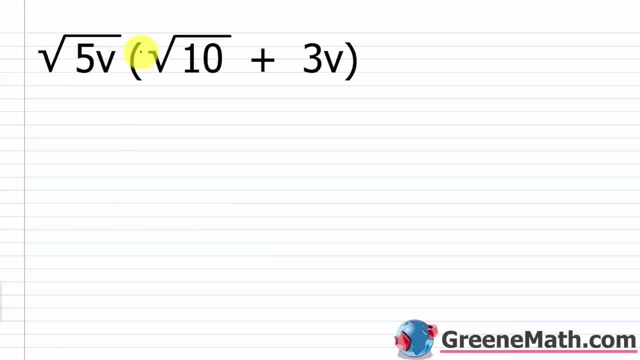 simple. And let's start out with the square root of 5v times the quantity, the square root of 10 plus 3v. So what I'm going to do here? because these are not able to be combined inside the parentheses here, I'm going to use my algebra. I'm going to use my algebra. I'm going to use my. 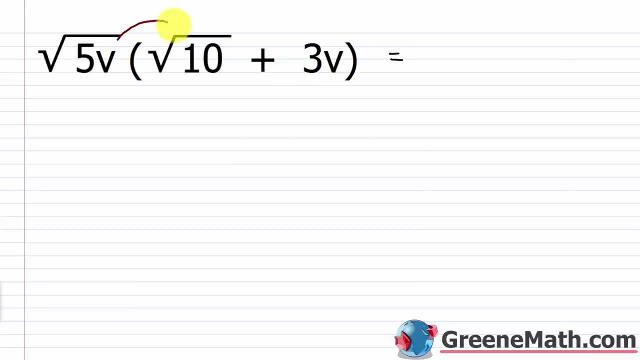 distributive property to simplify. So I'm going to multiply this, times this and also times this. We're going to see what we can simplify. So we'll have the square root of 5v multiplied by the square root of 10, and then plus the square root of 5v multiplied by 3v. Now can I do anything? 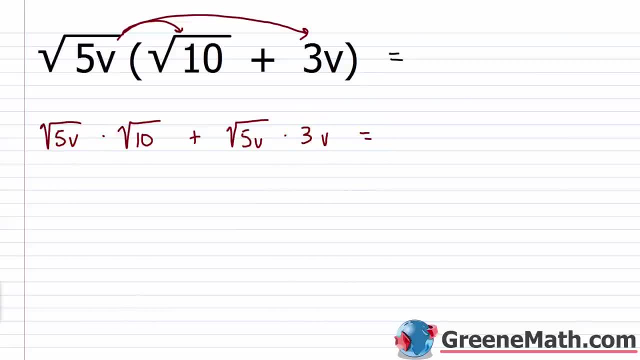 Well, yes, I can. The square root of 5v times the square root of 10, I can write that as what: the square root of 5v times the square root of 10. I can write that as what: The square of 5 times 10.. Think about breaking this down completely: Square root of 5 times square root. 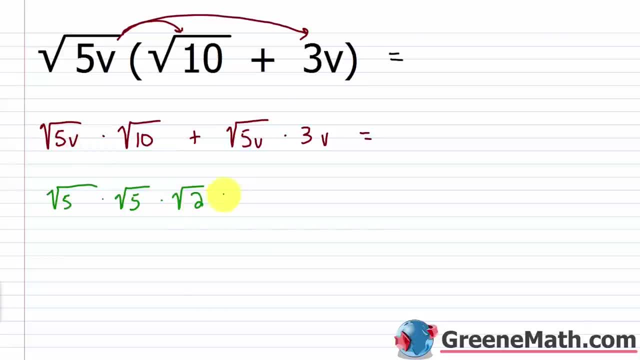 of 5 times square root of 2, and then times square root of v, Then plus Over here the square root of 5v. I could break that down, but really I'm not going to be able to do anything with that. 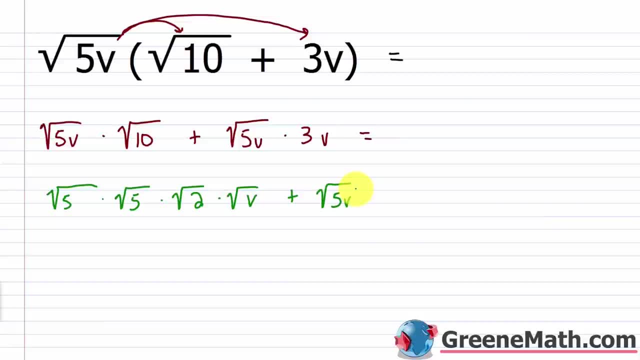 5 is prime. v is to the first power. nothing I can really do So. then times 3v. I can do stuff here, because the square root of 5 times the square root of 5 is 5.. So I can simply write that. 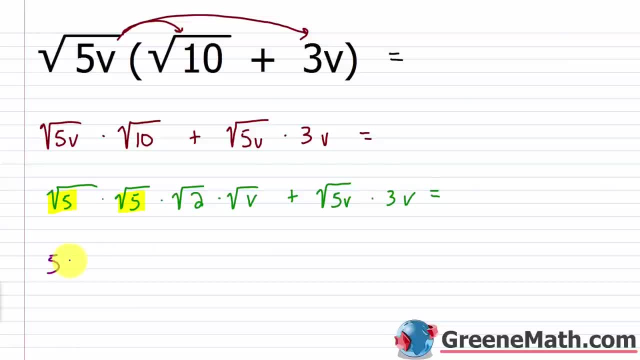 and say I have 5 times the square root of what's left, Square root of 2 times square root of v. we combine that and say we have the square root of 2v, then plus, I have the square root of 5v. 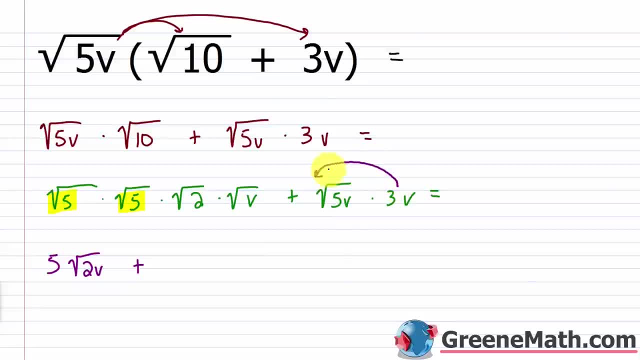 times 3v- Nothing I can do. so I just kind of change the order and I put 3v out in front. that's more traditional times, the square root of 5v. Now, is there anything else I can do? to simplify, I want you to think back to when we added and: 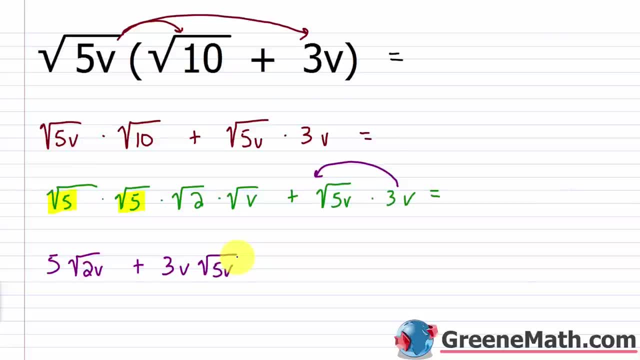 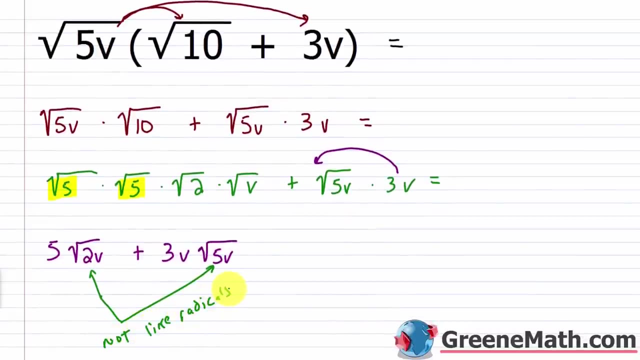 subtracted radicals We had to have like radicals. okay, These are not like radicals, If I look at this guy right here and I look at this guy right here. they're not like radicals. Why, Well, they have to have the same index, which, in this case, they're each square roots. 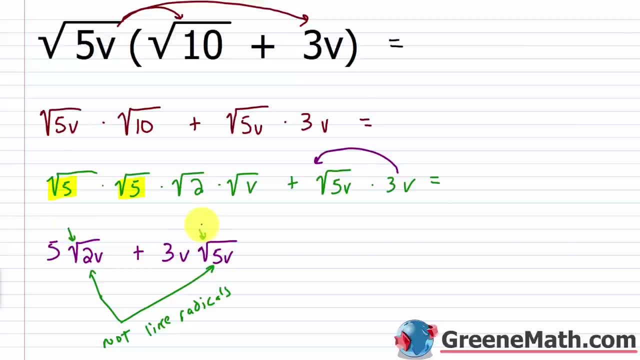 so that's a check. But then they have to have the same radicand. This is a 2v and this is a 5v. Those are not the same, okay. So they're not like radicals, Where students get confused on this is they're used to. 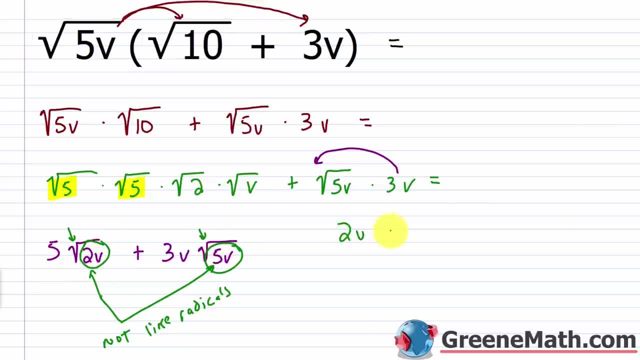 looking at like terms. So if I had 2v plus 5v- those are like terms- I can combine that and get 7v. But that's not the case here. It doesn't work that way with radicals, For, like radicals, 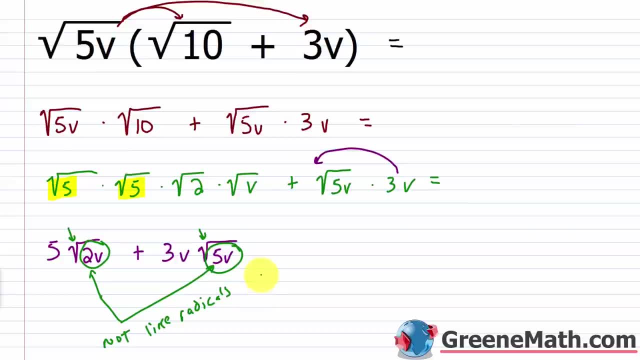 you have to have the exact same radicand. So if this was 5v and this was 5v, you're good to go. But in this case we have 2v and 5v, not good to go. So we don't have like radicals. So our simplified answer here is just 5 times. 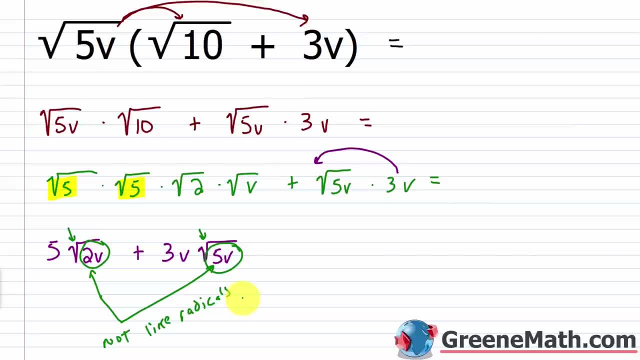 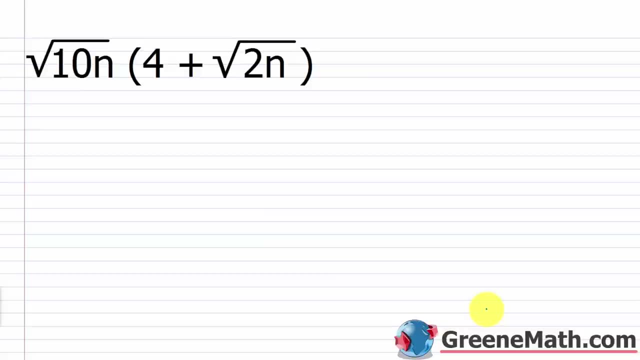 the square root of 2v plus 3v times the square root of 5v. All right, let's take a look at another one. So we have the square root of 10n times the quantity 4 plus the square root of 2n. 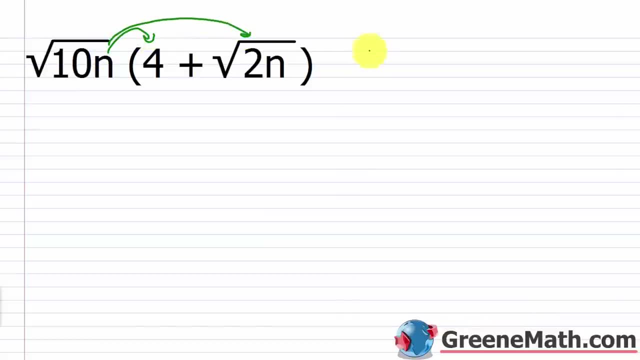 So again, I'm going to use my distributive property here and I'm going to start out the square root of 10n times 4, then plus the square root of 10n times the square root of 2n. So in this first case there's not going to be anything I can do to simplify. 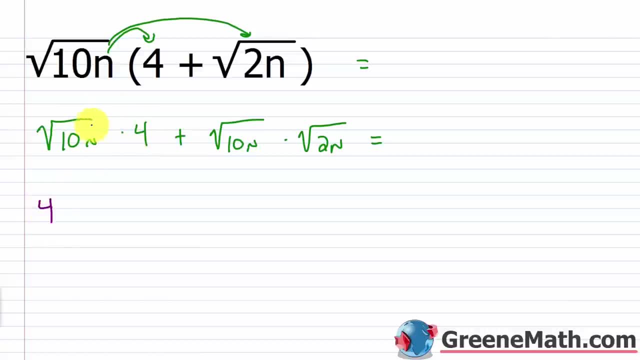 Why? Because I have a 4 out in front. I'm just going to switch the order of that to make it more traditional. Underneath the square root symbol, I have a 10. That factors in a 5 times 2.. 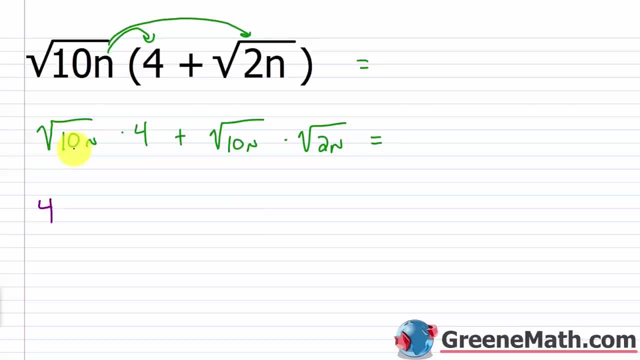 There's no perfect square in there right, So there's nothing I can do. Then I just have n. that's n to the first, Nothing I can do there. So this first part here, or the part on the left, will just be 4 times. 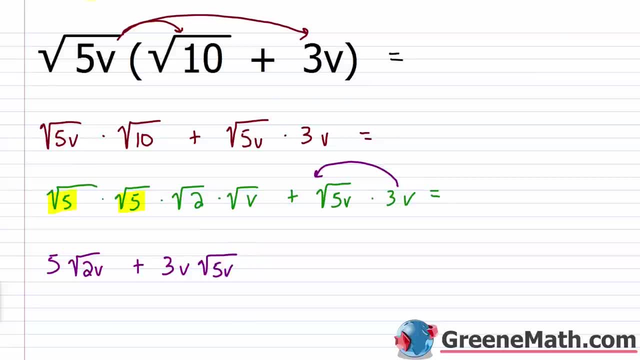 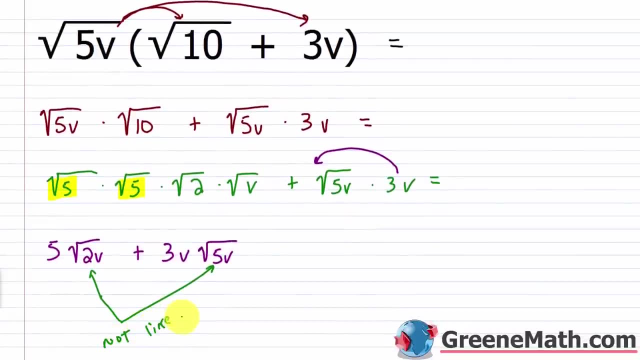 Okay? These are not like radicals. If I look at this guy right here, and I look at this guy right here, they're not like radicals. Why? Well, they have to have the same index, which in this case they're each square roots, so that's a check. But then they have to have the same radicand. This is a 2v, and this is a 5v. Those are not the same, okay? So they're not like radicals. Where students get confused on this, is when they get confused on the radicals, they're not like radicals. So, if you 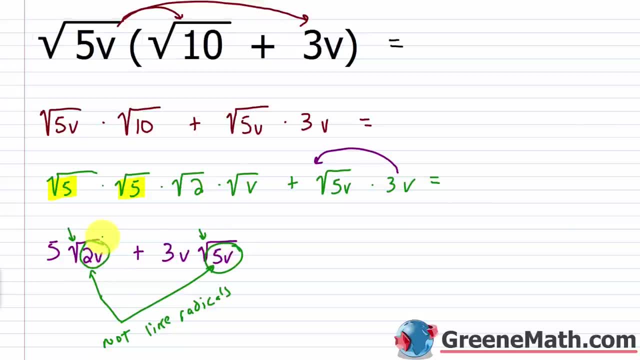 used on this is they're used to looking at like terms. So if I had 2V plus 5V, those are like terms. I can combine that and get 7V. But that's not the case here. It doesn't work that way with radicals. For like radicals, you have to have the exact same radicand. So if this was 5V and this was 5V, you're good to go. But in this case, we have 2V and 5V, not good to go. So we don't have like radicals. So our simplified answer here is just 5 times the square root of 2V plus 3V times 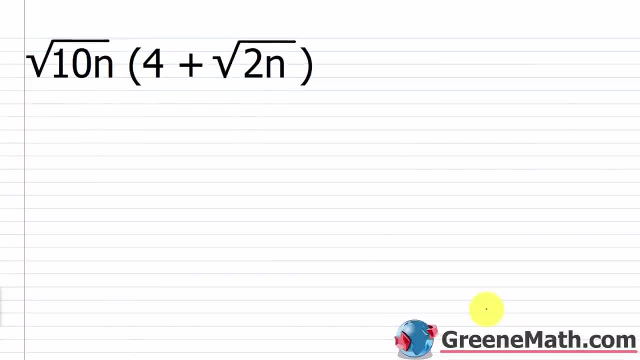 the square root of 5V. All right, let's take a look at another one. So we have the square root of 10N times the quantity 4 plus the square root of 2N. So again, I'm going to use my distributive property here. And I'm going to start out with the square root of 10N times 4, then plus the square root of 10N times the square root of 4. 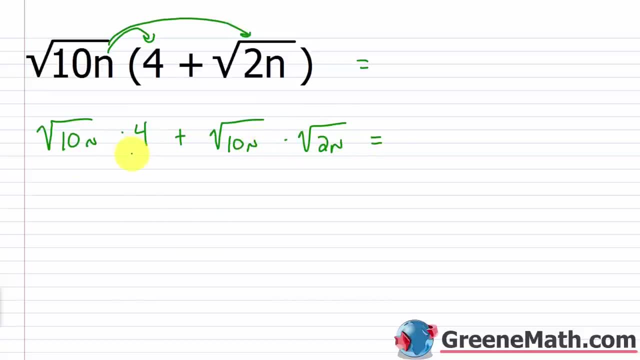 So in this first case, there's not going to be anything I can do to simplify. Why? Because I have a 4 out in front. I'm just going to switch the order of that to make it more traditional. Underneath the square root symbol, I have a 10. That factors in a 5 times 2. There's no perfect square in there, right? So there's nothing I can do. Then I just have N, that's N to the first power, nothing I can do there. So this first part here, the part on the left will just be 4 times the square root of 10N. 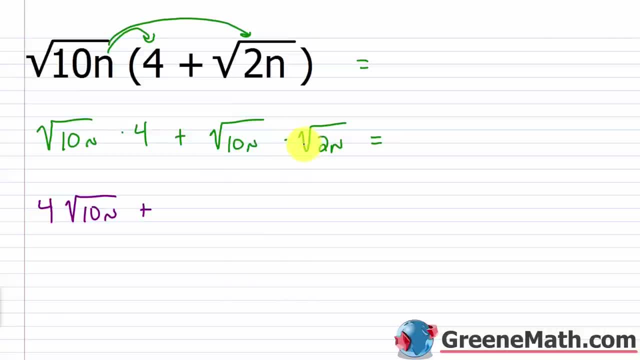 There's not going to be anything else I can do. Then plus. Here, there's going to be something I can do. Let's completely break this down. Let's say I have the square root of 10 is 5 times 2. So square root of 5 times square root of 2 times square root of that N there. 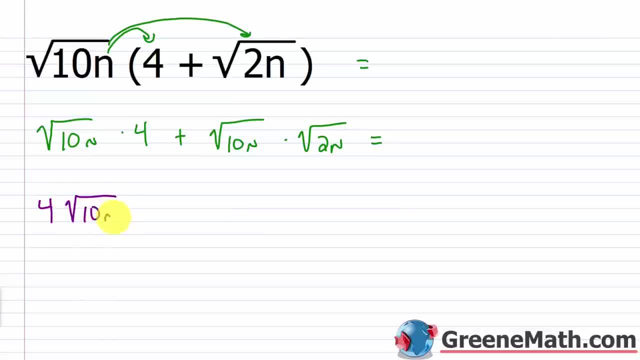 the square root of 10n, Nothing else I can do. Then, plus Here, there's going to be something I can do. Let's completely break this down. Let's say I have the square root of 10 is 5 times 2.. 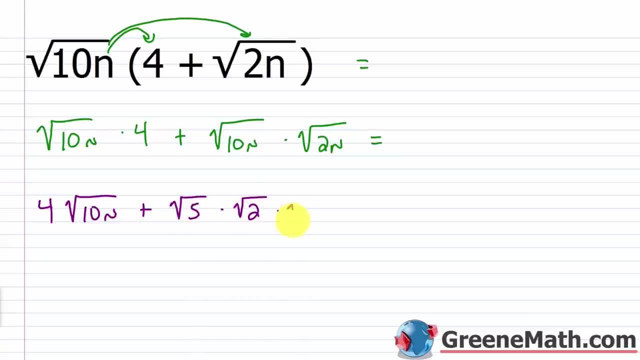 So square root of 5 times square root of 2 times square root of- I have that n there- 10 times Square root of 2n. I'm going to write square root of 2 times square root of n. Now what I have here is I have square root of 2 times square root of 2, and I also have 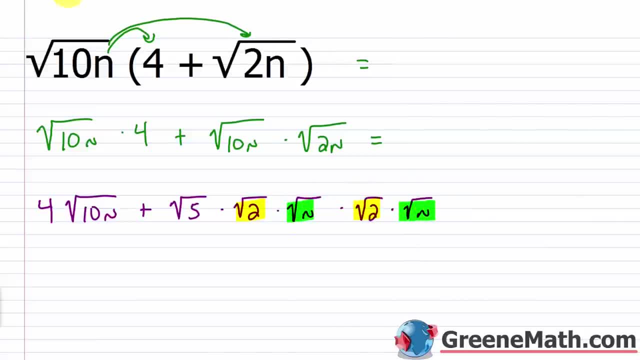 square root of n and square root of n. So what I want to do, let me report this first part. So 4 times square root of 10n plus square root of 2 times square root of 2 is 2.. Square root of n times square root of n is going to be n, So I'd have 2n there And then 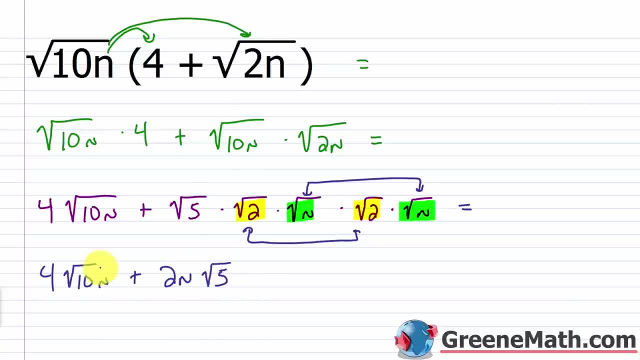 what's left? Just the square root of 5.. Let me kind of extend this a little bit, And these are not like radicals and I can't simplify any further, So I'm just going to report my answer as 4 times the square root of 10n plus 2n times the. 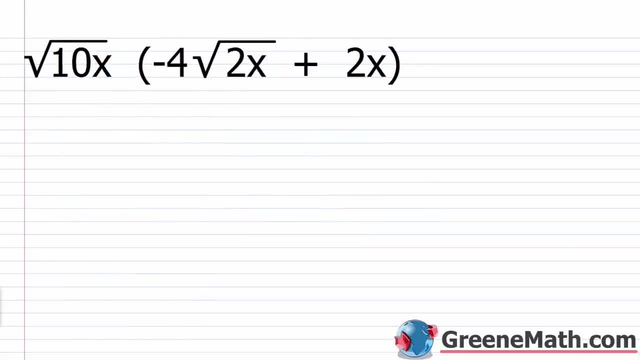 square root of 5.. All right, so for the next one, I have the square root of 10x times the quantity negative, 4 times the square root of 2x plus 2x. So again, I'm going to use my distributive. 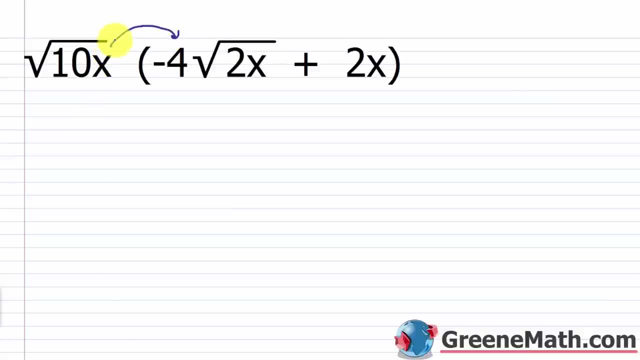 property here. So this times this and then plus this times this. All right, so we're going to have that negative 4 out in front times, the square root of 10x times the square root of 2x. Then plus I'm going to have, I'm going to put 2x out in front times the. 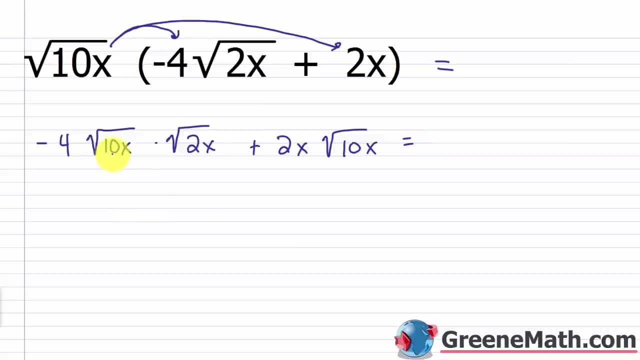 square root of 10x. Now, if I think about 10, again, it's 5 times 2.. So I know that I'm going to have 1.. I'm going to have a 2 here and a 2 here, So a pair of 2s- 1, 2- comes out right I. 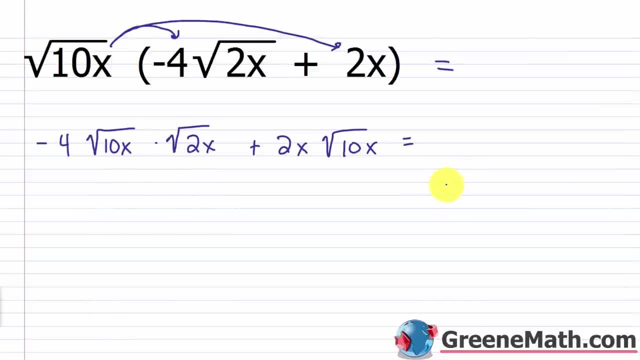 can kind of write it in a different way. Remember we looked at that in the previous lesson where we first started learning how to simplify. So if I did negative 4 out in front times, the square root of I'm going to go ahead. 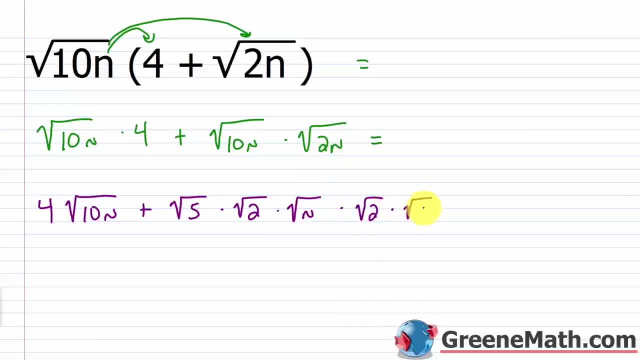 Then times. Square root of 2N, I'm going to write square root of 2 times square root of N. Now, what I have here is I have square root of 2 times square root of 2, and I also have the square root of N, and square root of N. what I want to do, let me report this first part. So 4 times square root of 10n plus square root of 2 times square root of 2 is 2. Square root of n times square root of n is going to be n. So I'd have 2n there. And then what's left? Just the square root of 5. Let me kind of extend this a little bit. And these are not like radicals. And I can't simplify any further. So I'm just going to report my answer as 4 times the square root of 10n plus 2n times the square root of 5. All right. 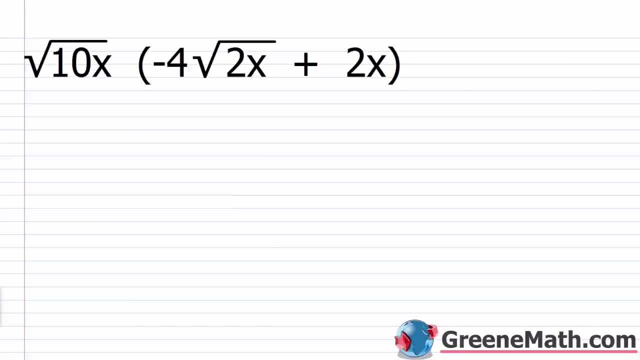 So for the next one, I have the square root of 10x times the quantity negative 4 times the square root of 2x plus 2x. So again, I'm going to use my distributive property here. So this times this and then plus this times this. All right. So we're going to have that negative 4 out in front times the square root of 10x times the square root of 2x. 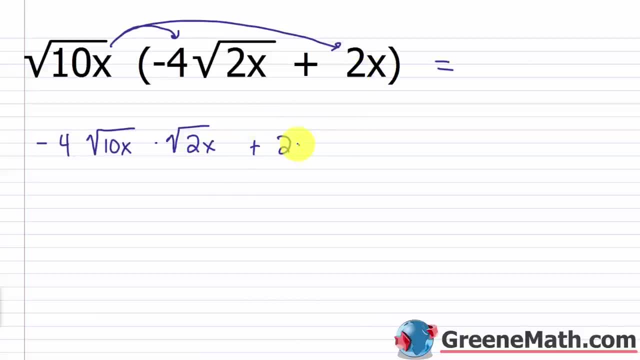 Then plus, I'm going to have, I'm going to put 2x out in front times the square root of 10x. Now, if I think about 10, again, it's 5 times 2. So I know that I'm going to have 1. I'm going to have a 2 here and a 2 here. So a pair of 2s, 1, 2 comes out. All right. I can kind of write it in a different way. Remember, we looked at that in the previous lesson where we first started learning how to simplify. So if I did negative 4 out in front, times the square root of, I'm going to go ahead and write this as 2 times 2. I've got a 2 here and I've got a 2 when I factor 10. And then times 5 and then times x times x. So I can think about it like that. And then plus 2x times the square root of, 10 factors into 5 times 2, but I don't really want to do it there because it's not going to help me. Let's just leave it as 10. And then x, I'm not going to factor that. I can't, I can't do anything with that. It's just x. Okay. So then each pair here, I'm going to pull one out, right? So 2 times 2, square root of 2 times square root of 2 is 2. So for each pair, 1 comes out. And then if I have x times x here, 1x will come out. Square root of x times square root of x is x. So I'd have negative 4 times, again, one of these is going to come out. One of these is going to come out. So negative 4 times 2 times x, and then times what's left under that square root symbol, which is 5. So times square root of 5. And then plus 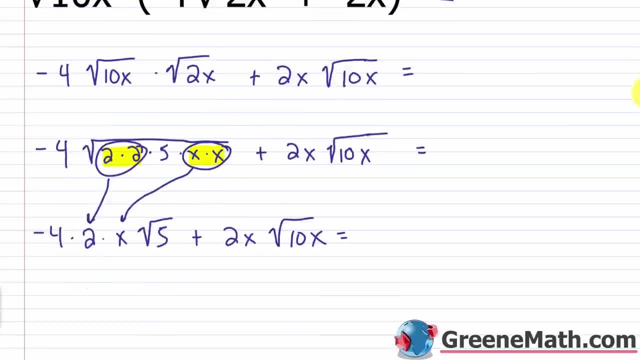 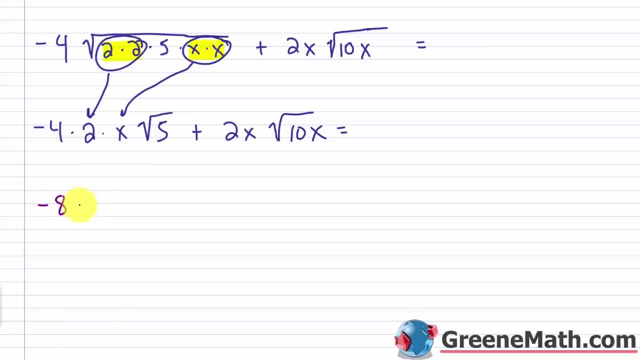 2x times square root of 10x. Let me scroll down here. So negative 4 times 2 is negative 8. So this would be negative 8 times x. So negative 8x. Then times square root of 5. Then plus 2x times square root of 10x. So that's going to be my simplified answer there. I don't have like 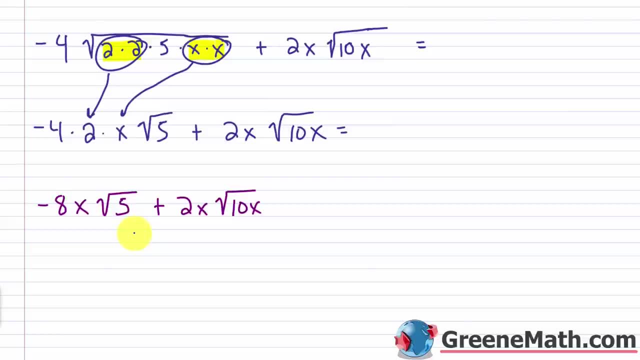 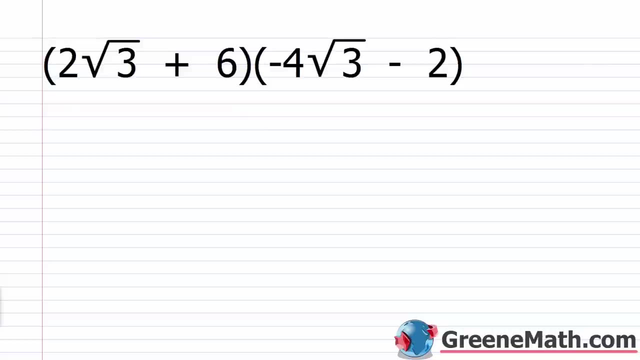 radicals. So there's nothing else I can do, right? Negative 8x times square root of 5 plus 2x times the square root of 10x. All right, let's get into something that's a little bit more complex. 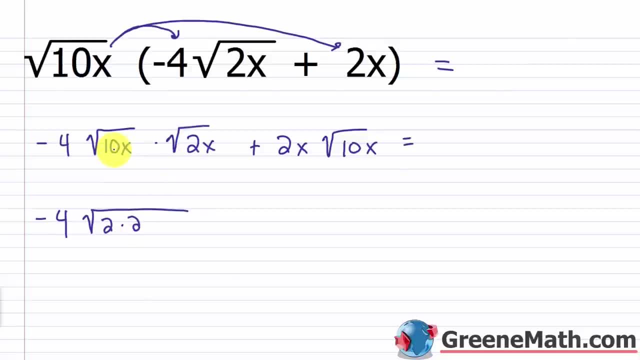 and write this as 2 times 2.. I've got a 2 here, and I've got a 2 when I factor 10.. And then times 5, and then times x, times x, So I can think about it like that- And then plus 2x times the square. 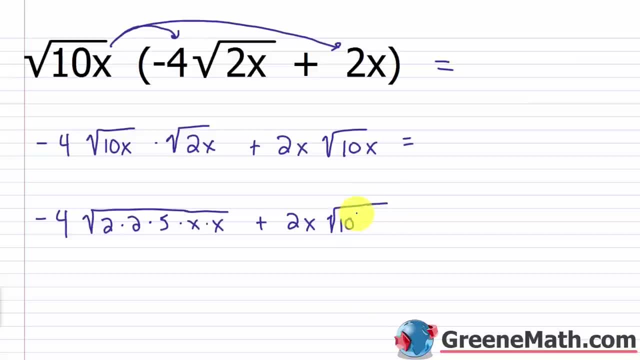 root of 10 factors into 5 times 2.. But I don't really want to do it there because it's not going to help me. Let's just leave it as 10.. And then x. I'm not going to factor that, I can't do. 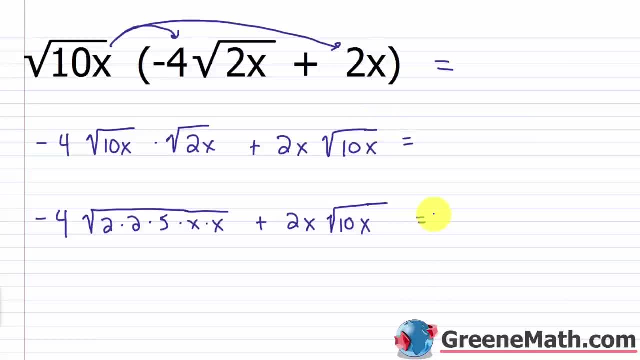 anything with that, It's just x. Okay, so then each pair here- I'm going to pull one out, right. So 2 times 2, square root of 2 times square root of 2 is 2.. So for each pair, 1 comes out, And then 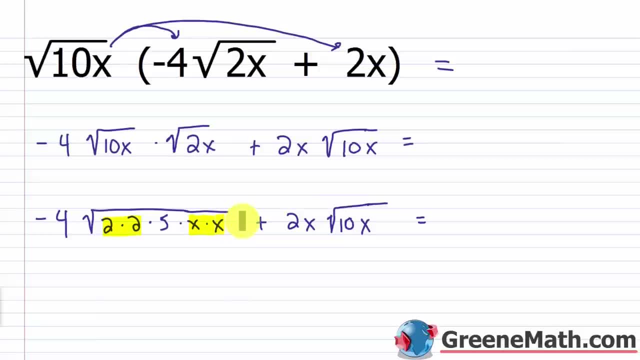 if I have x times x here, 1x will come out. Square root of x times square root of x is x, So I'd have negative 4 times again. one of these is going to come out. One of these is going to. 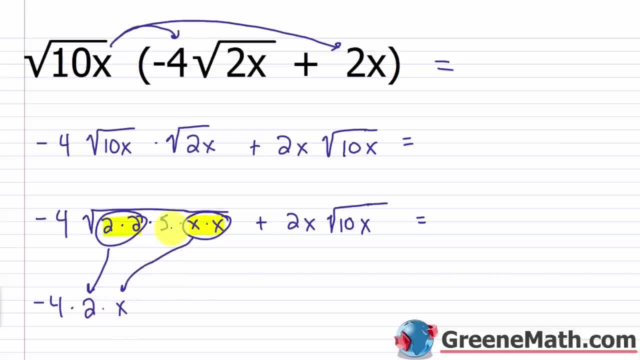 come out So negative 4 times 2 times x, and then times what's left under that square root symbol which is 5.. So times square root of 5. And then plus 2x times square root of 10x. 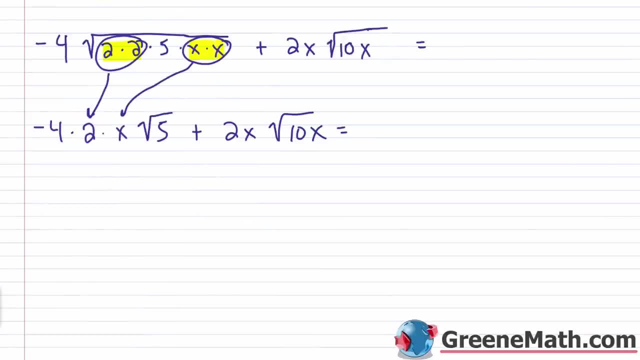 Let me scroll down here. So negative 4 times 2 is negative 8.. So this would be negative 8 times x. So negative 8x Then times square root of 5.. Then plus 2x times square root of 10x. 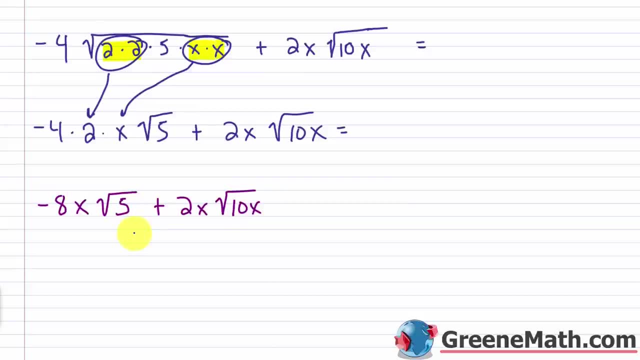 So that's going to be my simplified answer there. I don't have like radicals, So there's nothing else I can do. right? Negative: 8x times square root of 5 plus 2x times the square root of 10x. All right, let's get into something that's a little bit more complex. 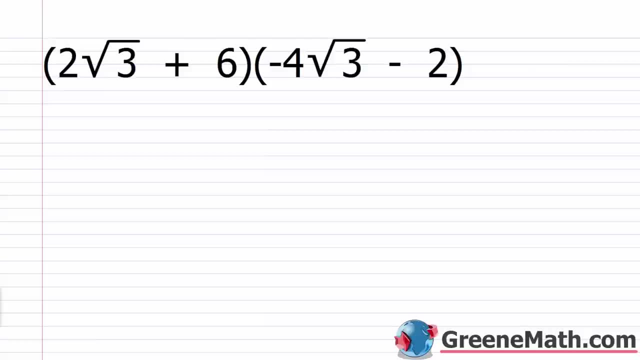 So I have the quantity 2 times square root of 3 plus 6 times the quantity negative, 4 times square root of 3 minus 2.. So the way we're going to do an operation like this, we're going to use FOIL, just like when we multiply two binomials together. right, We have two terms here and two. 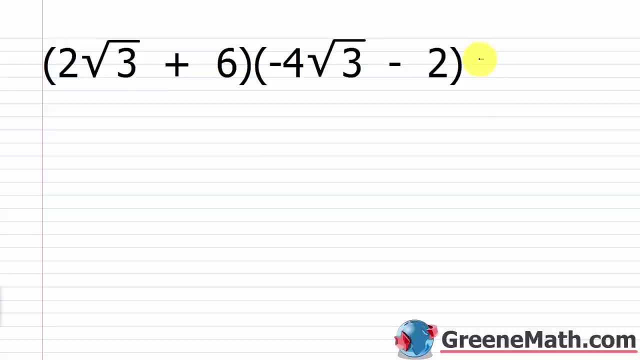 terms here, So let's use FOIL. So I'm going to do my first terms. So this guy times this guy 2 times negative. 4 is negative 8.. Square root of 3 times square root of 3 is 3.. So I'd have. 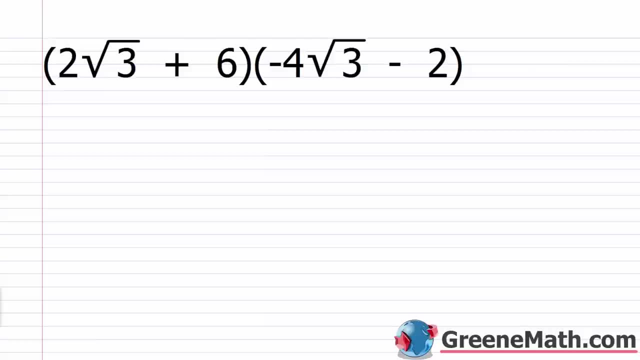 So I have the quantity 2 times square root of 3 plus 6 times the quantity negative 4 times square root of 3 minus 2. So the way we're going to do an operation like this, we're going to use FOIL, just like when we multiply two binomials together, right? We have two terms here and two terms here. So let's use FOIL. So I'm going to do my first terms. So this guy, this guy, 2 times negative 4 is negative 8. Square root of 3 times square root of 3 is 3. So I'd have negative 8 times 3, which we know is negative 24. So let's go ahead and write that. Okay, 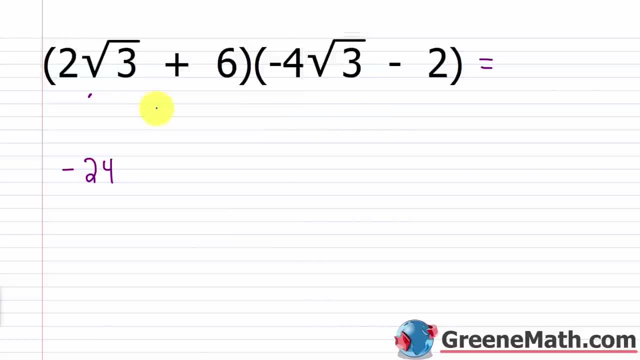 then the next thing I'm going to do is I'm going to multiply my outer terms. So this one times this one. So 2 times negative 2 would be negative 4. And then times that square root of 3. 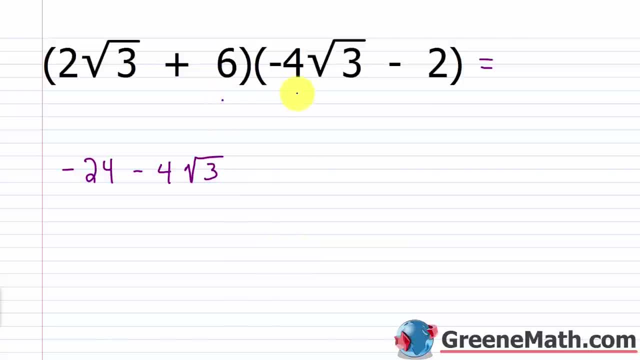 So now I'm going to multiply my inside terms. So this one times this one. 6 times negative 4 is negative 24. And then times square root of 3. And then lastly, I'm going to do my last terms. So 6 times negative 2 is negative 12. Okay, so once I have it in this format, pretty easy to simplify. 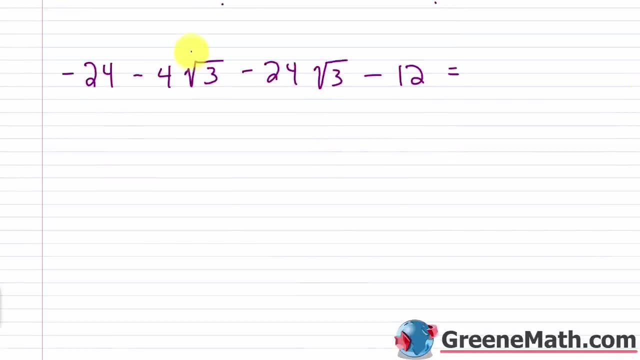 And in this case, we do have like radicals. We have the same index. We have the same index. We have the same radical. 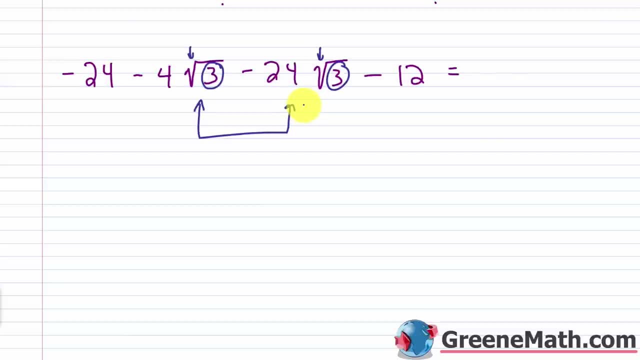 So we can combine what's in the middle. So if I look at negative 4 times square root of 3 minus 24 times square root of 3, negative 4 minus 24 is negative 28. So this would be negative 28 times that common radical, which is the square root of 3. Now negative 24 and negative 12 can also be combined. Negative 24 minus 12 is negative 36. So I can write negative 36 out in front or behind, doesn't matter. So we'd have negative 36, 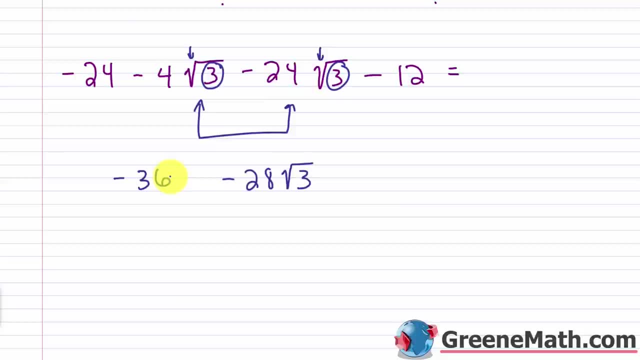 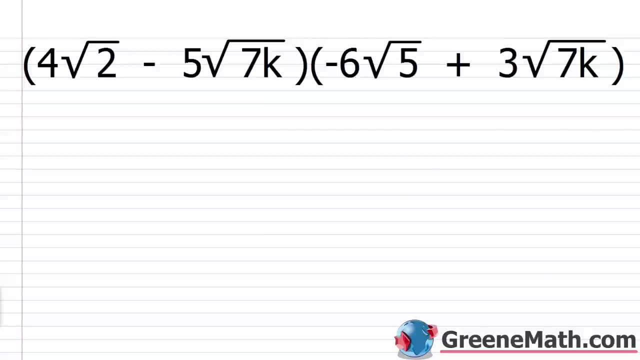 minus 28 times the square root of 3 as our answer. All right, for the next one, I have a similar situation. I have the quantity 4 times square root of 2 minus 5 times square root of 7k. And then this is multiplied by the quantity negative 6 times square root of 5 plus 3 times square root of 7k. 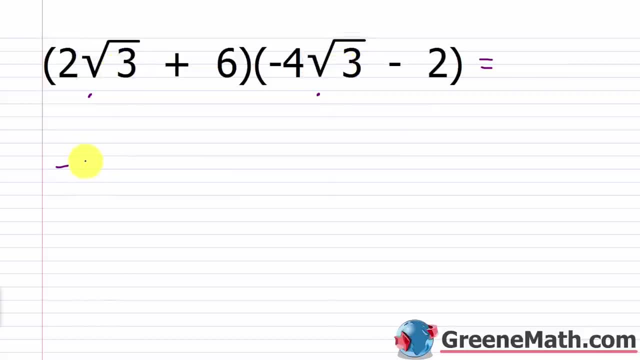 negative 8 times 3, which we know is negative 24.. So let's go ahead and write that. Okay, then the next thing I'm going to do is I'm going to multiply my outer terms. So this one times this one, So 2 times negative, 2 would be. 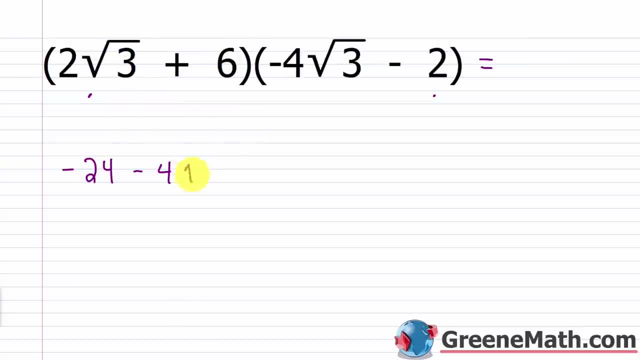 negative 4.. And then times that square root of 3.. So now I'm going to multiply my inside terms. So this one times this one, 6 times negative 4 is negative 24.. And then times square root of 3.. 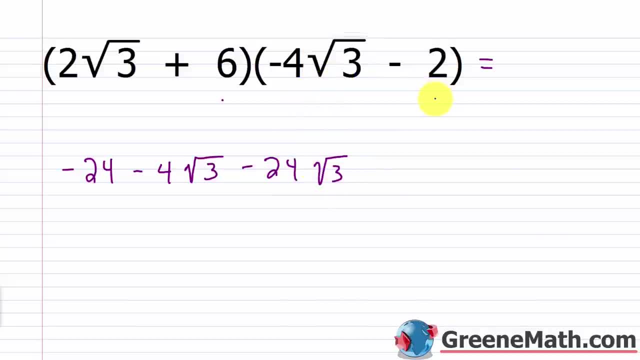 And then, lastly, I'm going to do my last terms. So 6 times negative 2 is negative 12.. Okay, so, once I have it in this format, pretty easy to simplify. And in this case we do have a negative 4.. So I'm going to do my last terms. 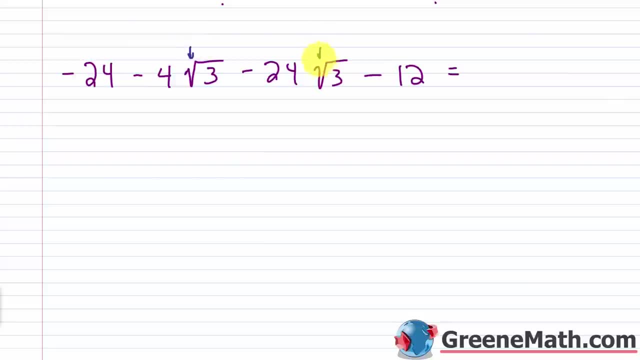 So we have, like radicals, We have the same index, We have the same index, We have the same radicand, So we can combine what's in the middle. So if I look at negative 4 times square root of 3 minus 24 times square root of 3, negative 4 minus 24 is negative 28.. So this would be: 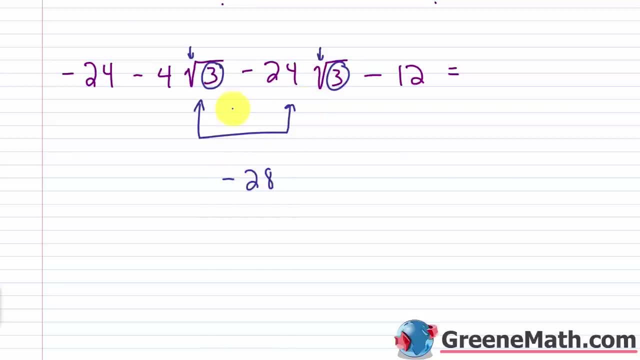 negative 28 times that common radical which is the square root of 3.. Now negative 24 and negative 12 can also be combined. Negative 24 minus 12 is negative 36.. So I can write negative 36 out, in front or behind, Doesn't matter. So we'd have negative 36. 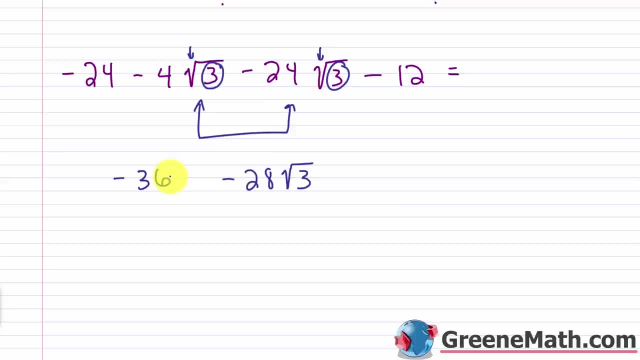 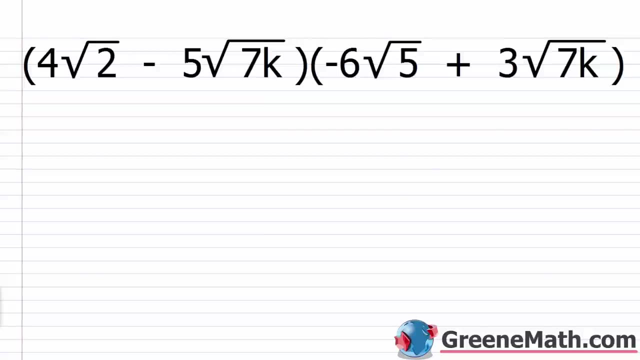 minus 28 times the square root of 3 as our answer. All right, for the next one, I have a similar situation. I have the quantity 4 times square root of 2 minus 5 times square root of 7k. 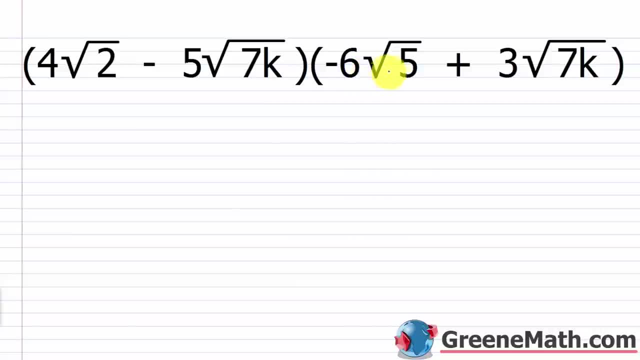 And then this is multiplied by the quantity negative 6 times square root of 5, plus 3 times square root of 7k. So again I'm going to use FOIL. So first terms: 4 times square root of 2, multiplied by negative 6 times square root of 5.. So 4 times negative 6 is negative 24.. 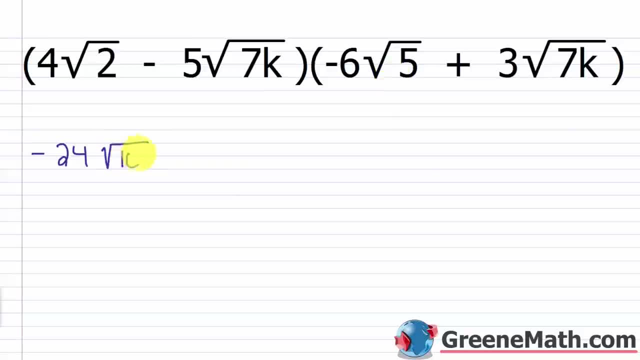 The square root of 2 times the square root of 5 is the square root of 10.. Now I want to do my outside terms. So I'd have 4 times square root of 2 times 3 times square root of 7k. So 4 times 3 would be 12, so plus 12.. Then the square root of 2 times the square 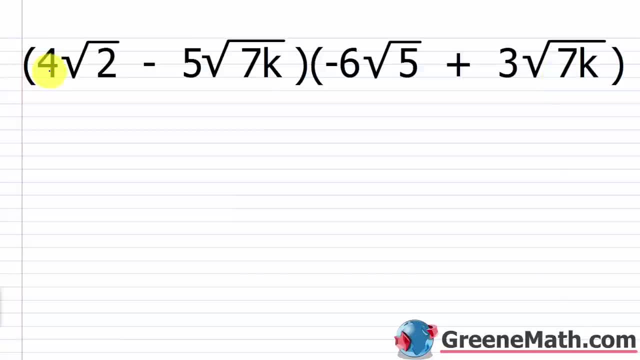 So again, I'm going to use FOIL. So first terms, 4 times square root of 2 multiplied by negative 6 times square root of 5. So 4 times negative 6 is negative 24. The square root of 2 times square root of 5 is the square root of 10. Now I want to do my outside terms. So I'd have 4 times square root of 2 times 3 times square root of 7k. So 4 times 3 would be 12, so plus 12. Then the square root of 2 times the square root of 7k would be the square root of 14k. Then my commuter terms, so I have negative 5 times square root of 7k multiplied by negative 6 times the square root of 5. so negative 5 times negative 6 is positive 30 and the square root of 7k times the square root of 5 would be the square root of 35k then I want to end by multiplying my last terms together so negative 5 times the square root of 7k times 3 times the square root of 7k so let's do negative times positive is negative 5 times 3 is 15 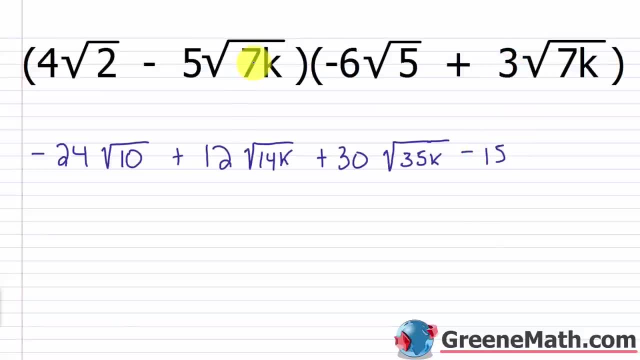 but then I've got square root of 7k times square root of 7k that's going to give me 7k so really I'd have negative 15 times 7 which is negative 105 times k so what can I simplify here? well the answer to that is nothing this is 14k, this is 35k that's not the same these are not like radicals very important that you understand so my simplified answer will just be negative 24 times square root of 10 plus 12 times the square root of 14k 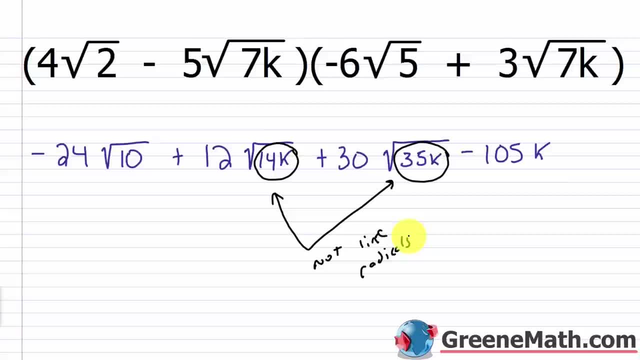 plus 30 times the square root of 35k minus 105k 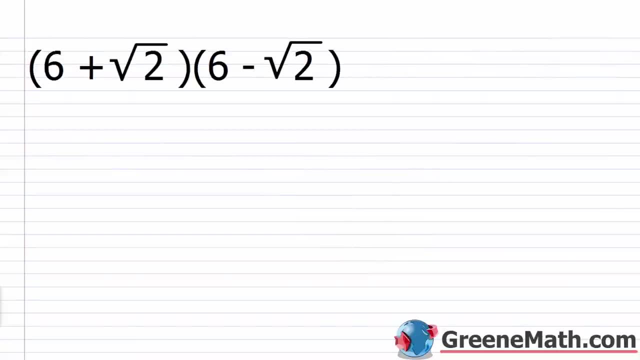 alright for the next one I want you to think back to when we saw the difference of two squares and we know the difference of two squares looks like this it's x squared minus y squared and when we factor it we end up with x plus y times x minus y those two quantities now what you'll see in this case is you have this right here and this right here as the same term and then this right here and this right here as the same term what's different would be the signs right you have a plus and a minus 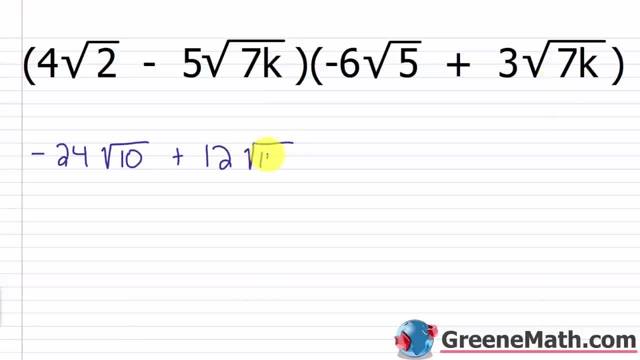 root of 7k would be the square root of 14k, Then my inner terms. So I have negative 5 times the square root of 7k multiplied by negative 6 times the square root of 5.. So negative 5 times negative 6 is positive 30.. And the square 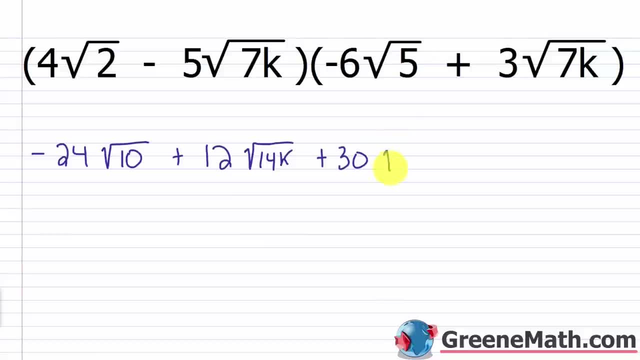 root of 7k times the square root of 5 would be the square root of 35k. Then I want to end by multiplying my last terms together, So negative 5 times the square root of 7k times 3 times the square root of 7k. So let's do. 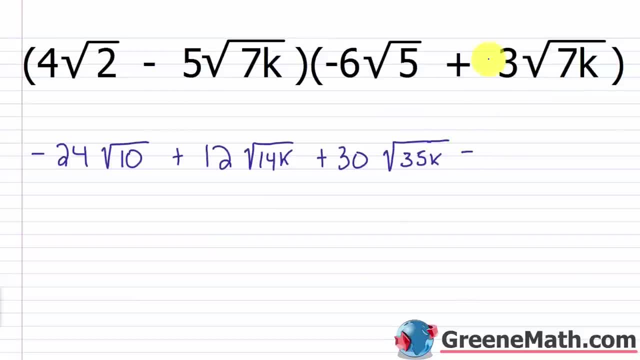 that Negative times positive is negative. 5 times 3 is 15.. Okay, 15.. But then I've got square root of 7k times square root of 7k. That's going to give me 7k. So really I'd. 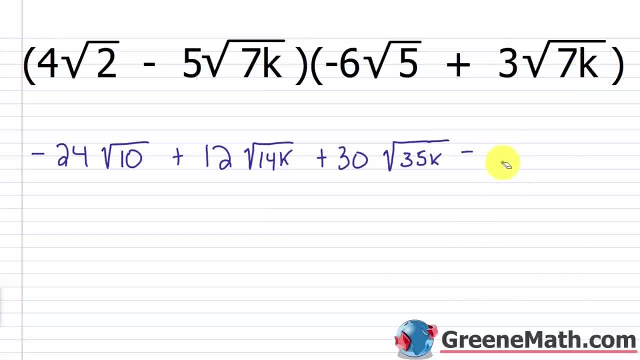 have negative 15 times 7, which is negative 105 times k. So what can I simplify here? Well, the answer to that is nothing. This is 14k, This is 35k. That's not the same, These are not. 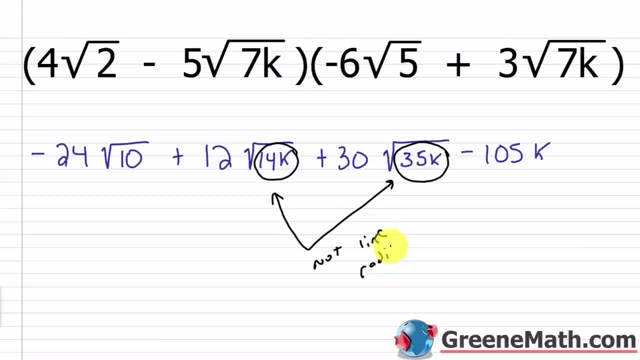 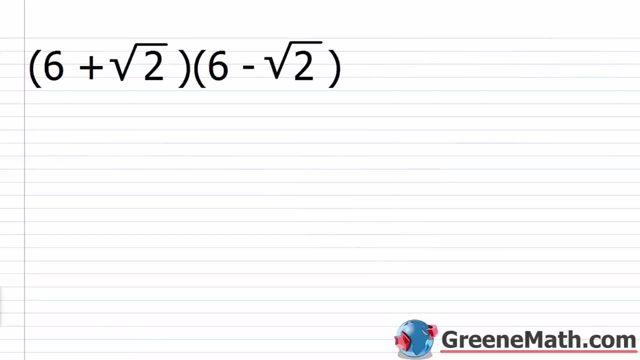 Not like radicals. Okay, very important that you understand that. So my simplified answer will just be negative: 24 times square root of 10 plus 12 times the square root of 14k plus 30 times the square root of 35k minus 105k. All right, for the next one I want you to think back to when we saw 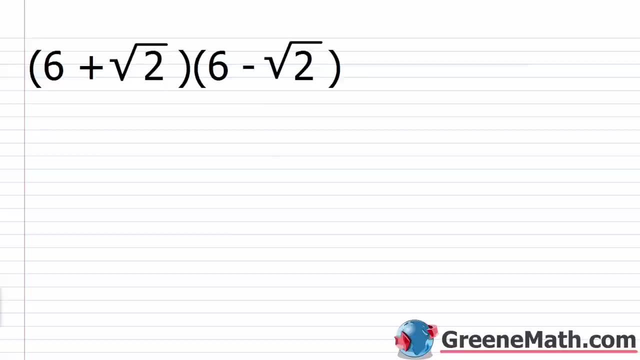 the difference of two squares, And we know. the difference of two squares looks like this: It's x squared minus y squared, And when we factor it, we end up with x plus y times, x minus y. right, Those two quantities. Now what you'll see in: 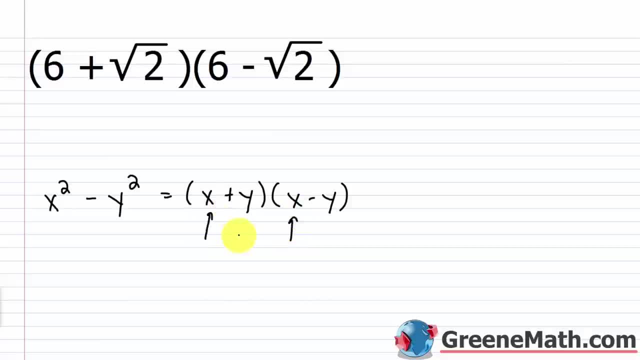 this case is: you have this right here and this right here as the same term, And then this right here and this right here as the same term. What's different would be the signs. right, You have a plus and a minus. Now look at what you have here. You have a 6 and a 6.. And then look over here. 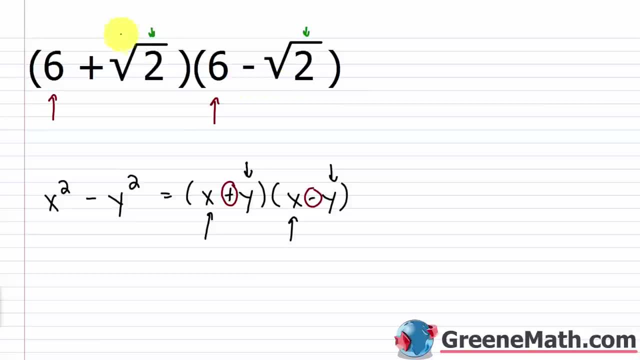 You have square root of 2 and square root of 2.. Then your signs are different. You have a positive and a negative. So they throw things at you, especially on timed examinations, to kind of say, okay, well, you should recognize this pattern And you should know that all I need. 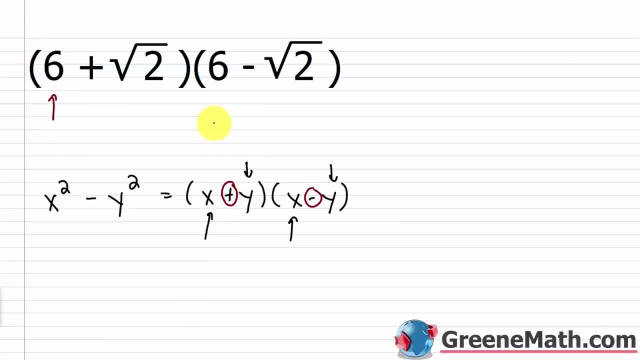 now look at what you have here you have a 6 and a 6 and then look over here you have square root of 2 and square root of 2 then your signs are different you have a positive and a negative so they throw things at you especially on timed examinations to kind of say okay well you should recognize this pattern and you should know that all I need to do is square this and then subtract away this square alright so really the answer I can just do this in my head 6 squared is 36 and then minus the square root of 2 squared would be 2 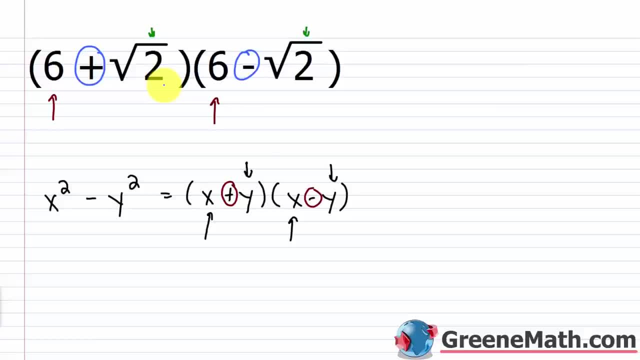 so 36 minus 2 would be 34 alright so that should be your answer 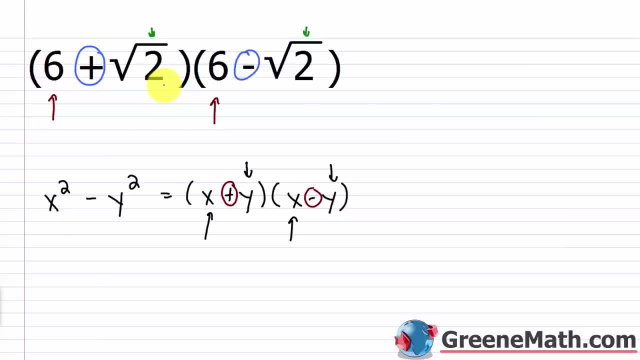 again you can do that in your head once you're familiar with this pattern 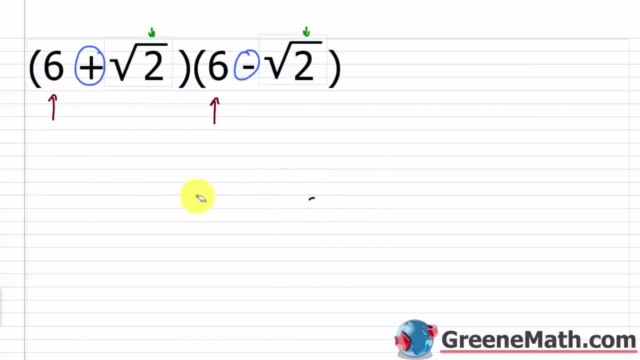 so let's go ahead and crank this out the long way and then again we'll do it the short way 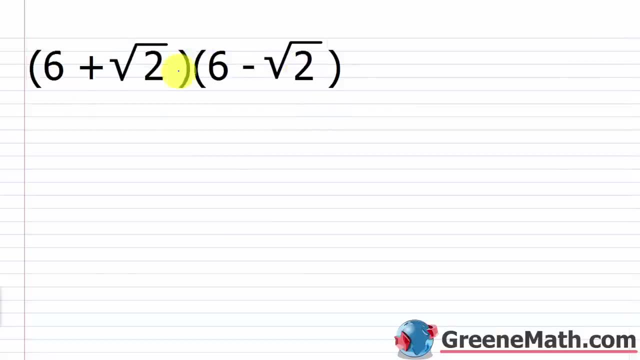 so if I was to use FOIL here so let's start with 6 times 6 that's 36 and then 6 times negative square root of 2 would be minus 6 times square root of 2 then next I have the square root of 2 times 6 so that's plus 6 times square root of 2 and then last I have square root of 2 times negative square root of 2 that's minus 2 right square root of 2 times square root of 2 is 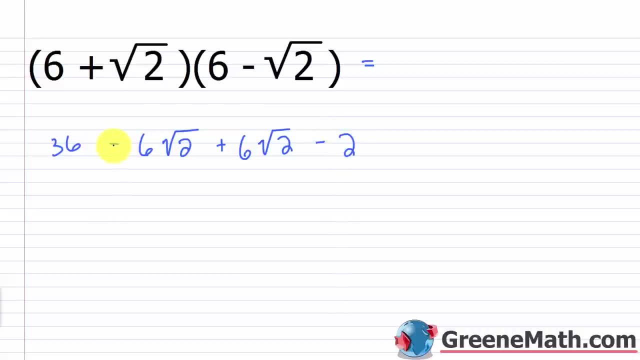 2 so now again we realize that the two terms in the middle here the negative 6 times square root of 2 and the positive 6 times square root of 2 those are going to cancel out and all I'm left with is the first term that we saw squared minus the second term that we saw squared right so it's 36 minus 2 which again is 34 and you saw me do that in my head and the reason I can do that in my head and you can too is because I recognize the pattern right away right so this ends up being a square root of 2 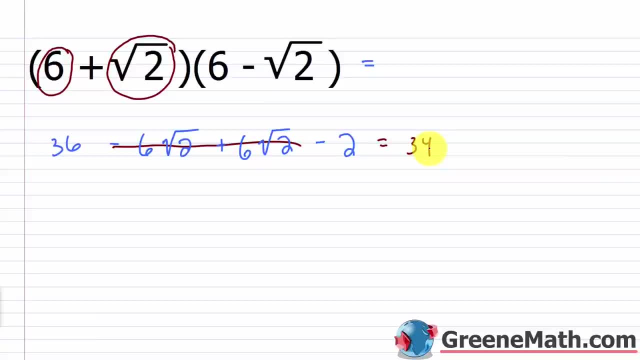 right so this ends up being a square root of 2 right so this ends up being a square root of 2 and again the quick way to do that is square the first thing square 6 that's 36 minus the second thing squared square root of 2 squared would just be 2 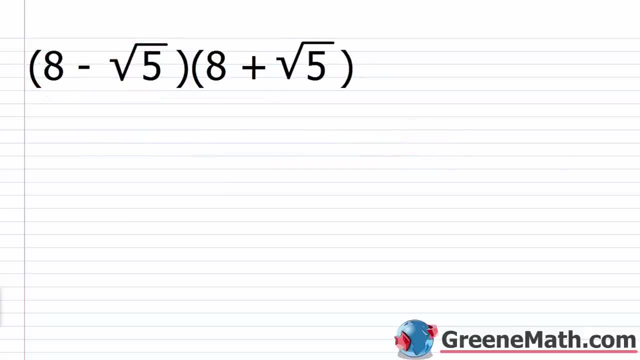 36 minus 2 is 34 right so here we have that same scenario 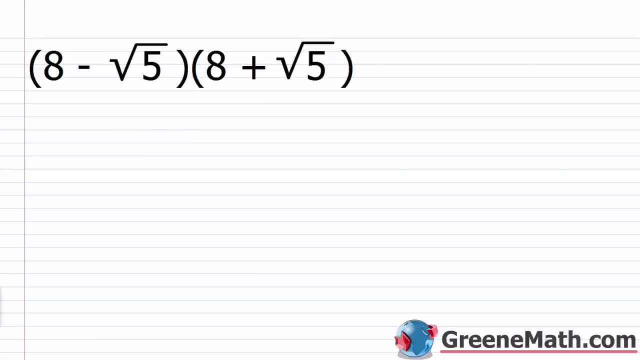 8 minus the square root of 5 that quantity times the quantity 8 plus the square root of 5 very easy to do this if you recognize it 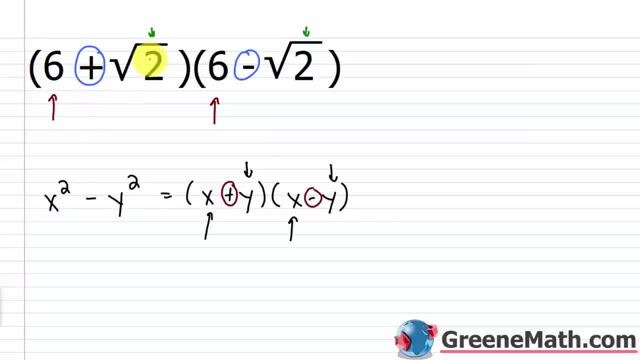 to do is square this and then subtract away this square, right. So really the answer- I can just do this in my head- 6 squared is 36.. And then minus the square root of 2 squared would be 2.. So 36 minus 2 would be 34, right. So that should be. 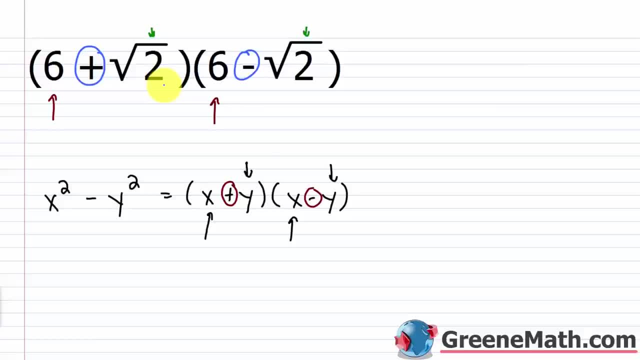 your answer. Again, you can do that in your head once you're familiar with this pattern. So let's go ahead and crank this out the long way And then again we'll do it the short way. So if I was to use FOIL here, so let's start with 6 times 6, that's 36. And then 6 times. 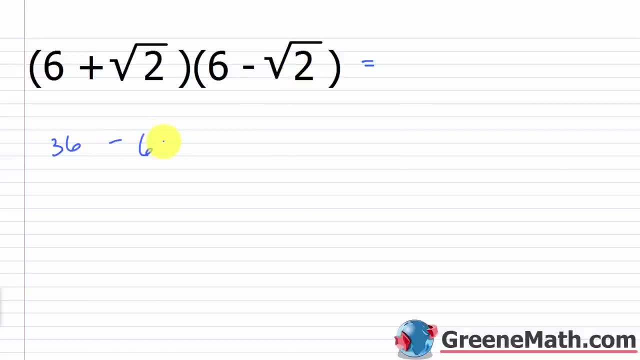 negative square root of 2 would be minus 6 times square root of 2.. Then next, I have the square root of 2 times 6. So that's plus 6 times square root of 2.. And then, last, I have square root of 2 times. 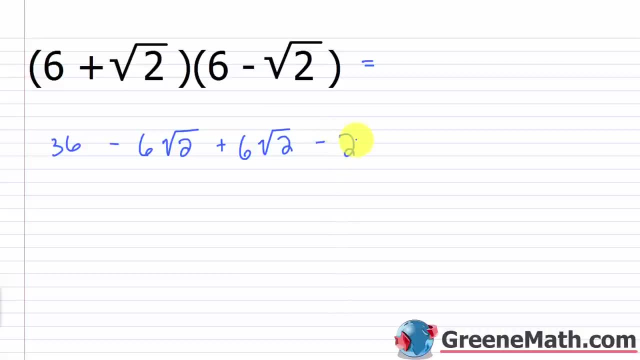 negative square root of 2.. That's minus 2, right Square root of 2 times square root of 2 is 2.. So now again we realize that the two terms in the middle here, the negative 6 times square root of 2 and the 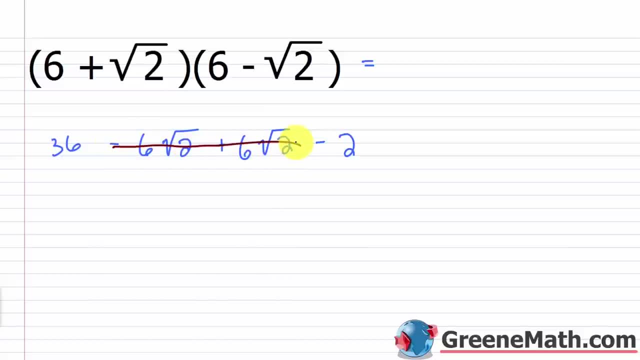 positive 6 times square root of 2, those are going to cancel out And all I'm left with is the first term that we saw squared minus the second term that we saw squared right. So it's 36 minus 2,. 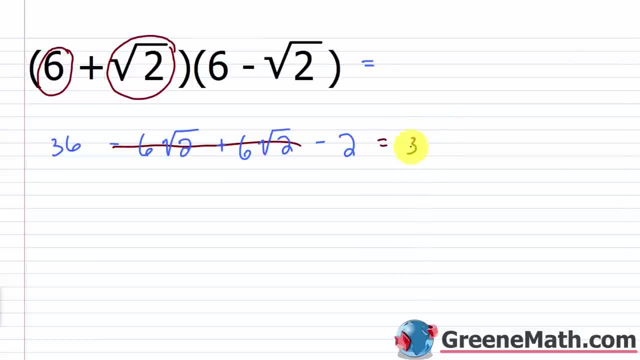 which, again, is 34.. And you saw me do that in my head, And the reason I can do that in my head too is because I recognize the pattern right away, right? So this ends up being 34.. And again. 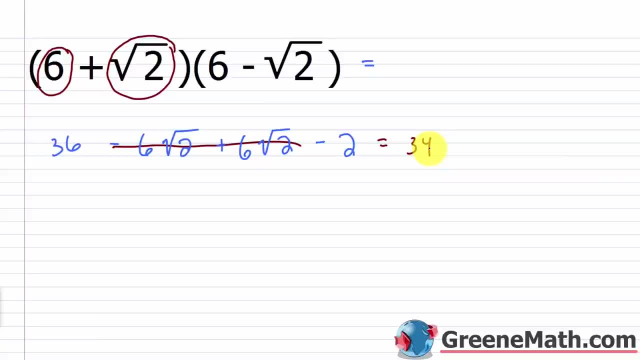 the quick way to do that is: square the first thing, square 6, that's 36, minus the second thing. squared square root of 2, squared would just be 2.. 36 minus 2 is 34.. All right, so here. 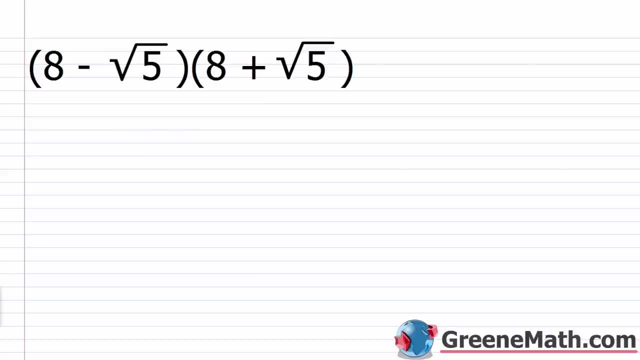 we have that same scenario: 8 minus the square root of 5, that quantity times the quantity 8 plus the square root of 5.. Very easy to do this, If you recognize it: you just square the first guy. So if I square 8, I get 64. Then, minus, square the second guy, Square root. 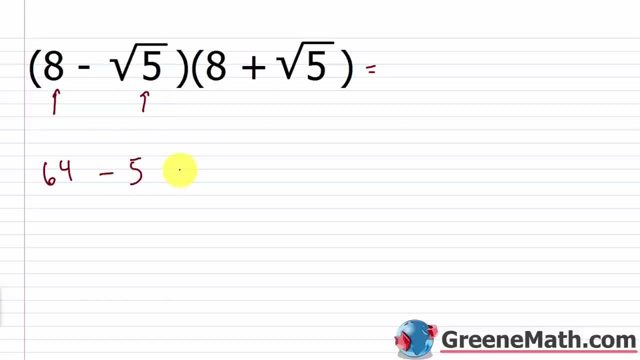 of 5 squared is 5.. So 64 minus 5 would be 59.. All right, we can do this the long way just to verify that we get that answer, but I'm going to promise you 100% of the time you will, So 8 times. 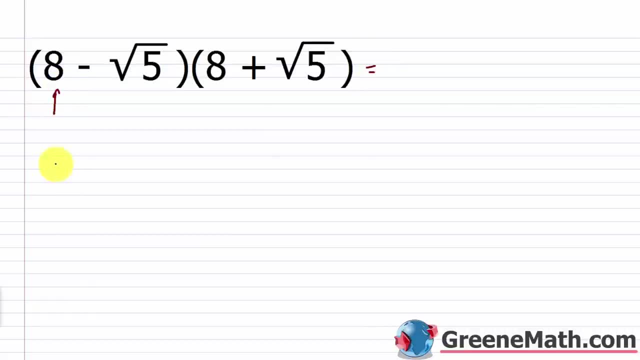 you just square the first guy so if I square 8 I get 64 then minus the first thing minus the square root of the second guy square root of 5 squared is 5 so 64 minus 5 would be 59 right and we can do this the long way just to verify that we get that answer but I'm gonna promise you 100% of the time you will so 8 times 8 would be 64 the outer would be positive 8 times square root of 5 then the inner 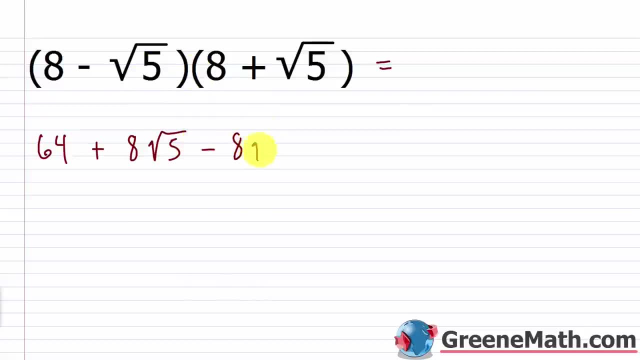 we'd have negative 8 times square root of 5 then the last negative square root of 5 times square root of 5 we know it's negative square root of 5 times square root of 5 is 5 so again the two terms in the middle are gonna drop out right those are just gonna cancel and I'm left with 64 minus 5 which again is 59 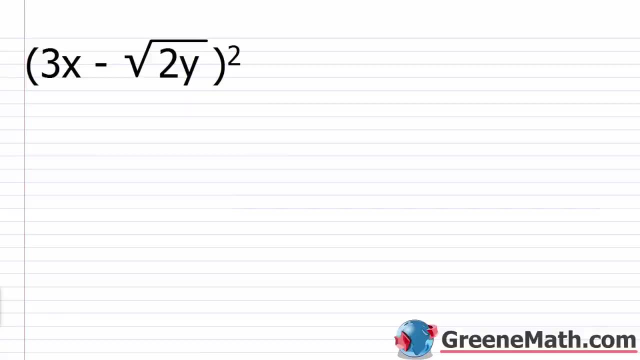 all right for the next one again we're gonna utilize our special products formulas so do you recall something like the quantity x minus y squared right you should know that 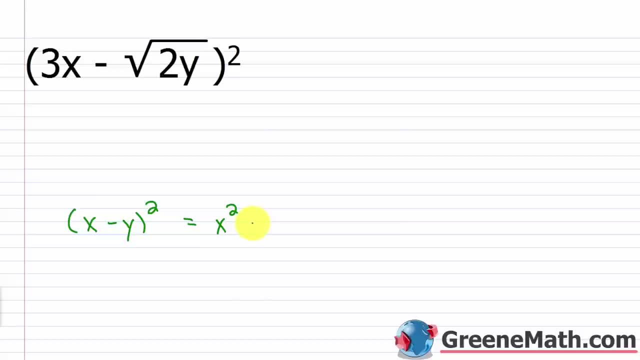 right you should know that you should be able to regurgitate this formula at this point it's x squared minus right because we have a minus there 2xy plus y squared 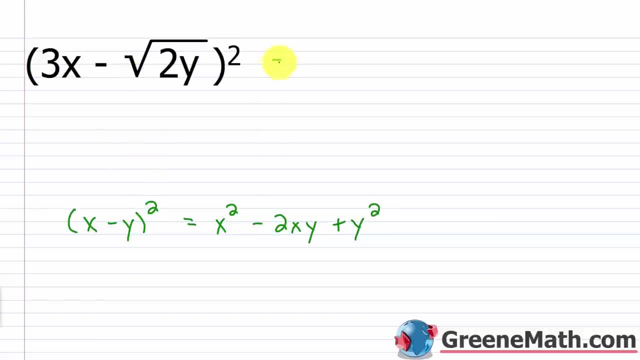 so following that format here I would have the first guy squared so 3x squared 3 squared is 9 x squared is just x squared I would have minus 2 times the first guy which is 3x times the second guy which is the square root of 2y and then I would have 2x squared and then plus the second guy squared 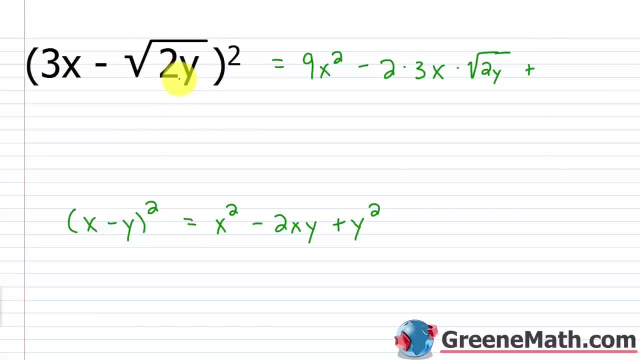 so the square root of 2y squared the squaring would just undo the square root I'm left with just 2y 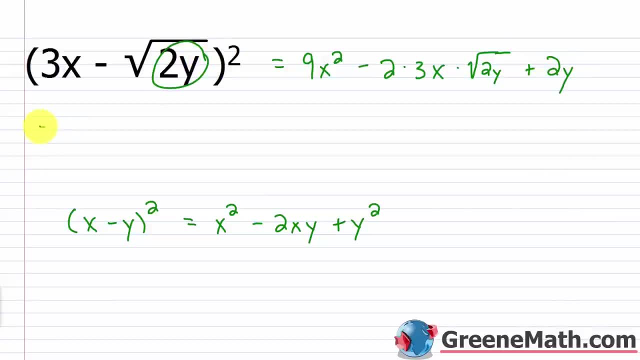 so plus 2y so if I simplify this I get what 9x squared minus 2 times 3 is 6 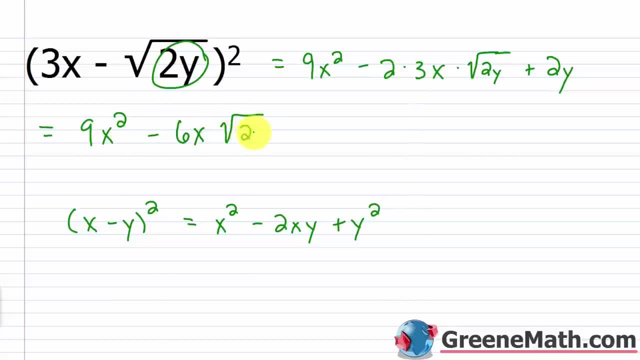 I'd have 6x times the square root of 2y and then plus 2y so that's as simple as I can get that I'm not gonna be able to further simplify because there's nothing to combine there. So I'm gonna go ahead and do that. 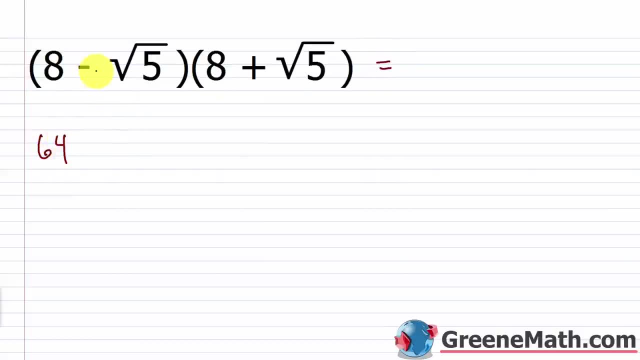 8 would be 64.. The outer would be positive 8 times square root of 5.. Then the inner. we'd have negative 8 times square root of 5.. Then the last negative square root of 5 times square root of 5.. We know it's negative Square root of 5 times. 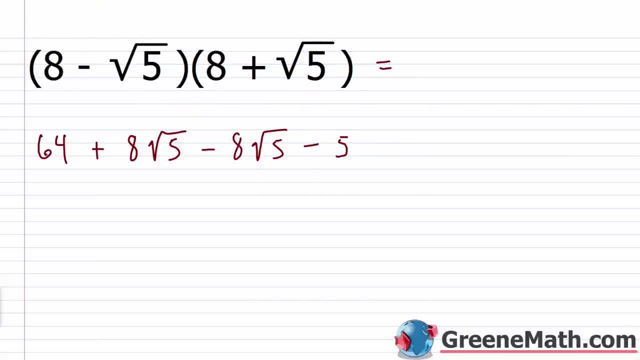 square root of 5 is 5.. So again, the two terms in the middle are going to drop out, right. Those are just going to cancel And I'm left with 64 minus 5, which again is 59.. All right, 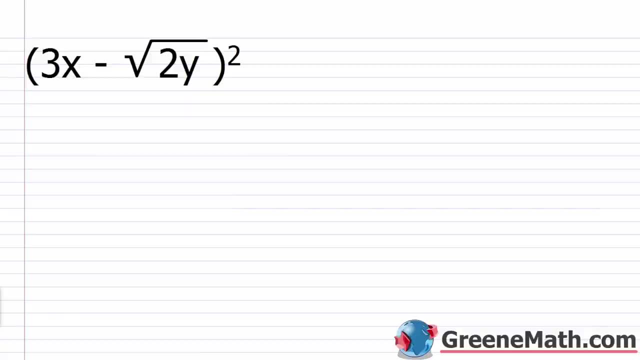 for the next one, again, we're going to utilize our special products formulas. So do you recall anything like the quantity x minus y squared? All right, you should be able to regurgitate this formula at this point. It's x squared minus, right, because we have a minus there: 2xy plus y. 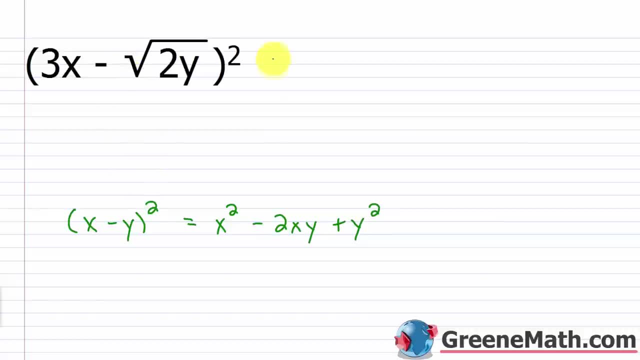 squared. So following that format here, I would have the first guy squared, So 3x squared, 3 squared is 9.. x squared is just x squared. I would have minus 2 times the first guy, which is 3x. 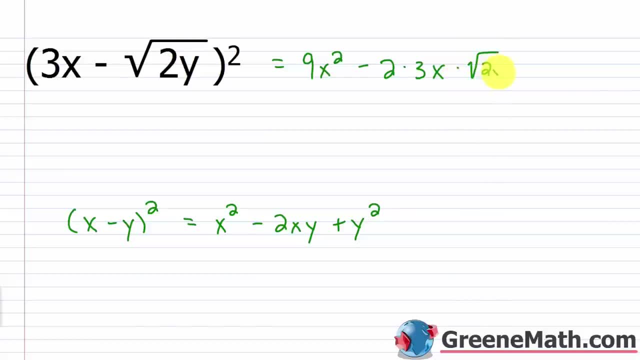 times the second guy, which is 3x. So I would have minus 2 times the first guy, which is 3x times the second guy, which is the square root of 2y, and then plus the second guy, squared So. 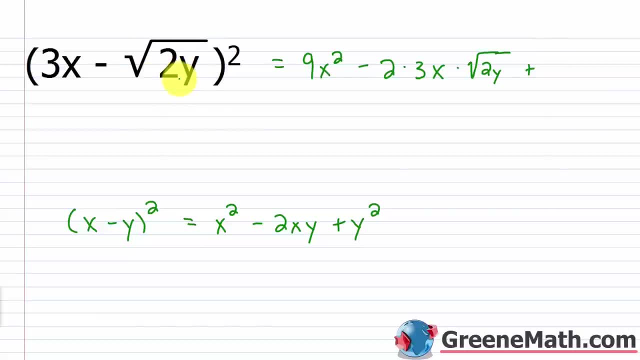 the square root of 2y squared. the squaring would just undo the square root. I'm left with just 2y, so plus 2y. So if I simplify this, I get what: 9x squared minus 2 times 3 is 6.. I'd have 6x. 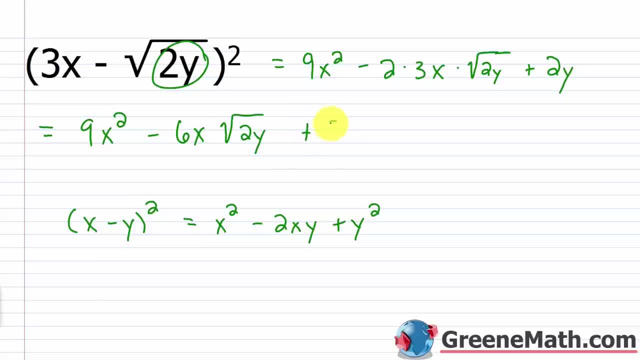 times the square root of 2y and then plus 2y. So that's as simple as I can get that. I'm not going to be able to further simplify because there's nothing to combine there. So I would just erase this here and show you. I get the same answer if I did it the long. 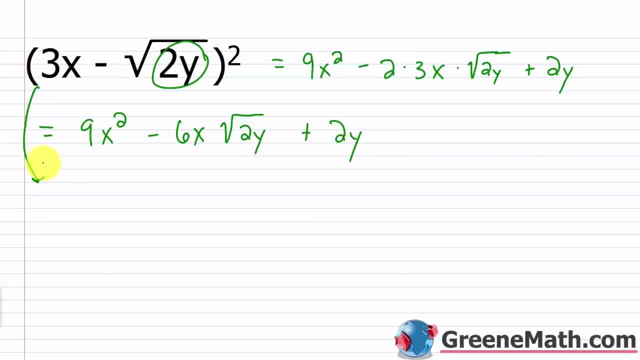 way. So remember, I need to expand this if I want to do it the long way. I would say this is 3x minus the square root of 2y And then, if this is squared, I would say this is 3x minus the square. 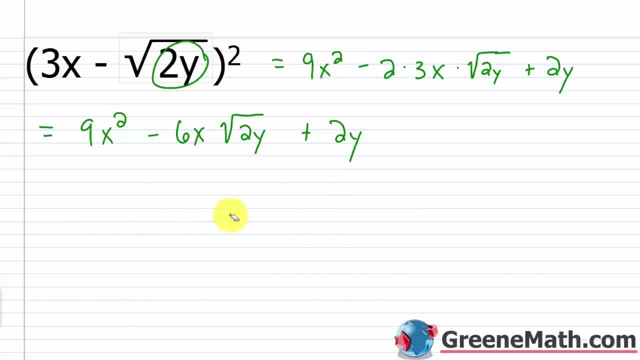 So I would just erase this here and show you I get the same answer if I did it the long way. So remember I need to expand this if I want to do it the long way I would say this is 3x minus the square root of 2y and then if this is squared I would say this is 3x minus the square root of 2y times again 3x minus the square root of 2y so the first terms 3x times 3x would be 9x squared 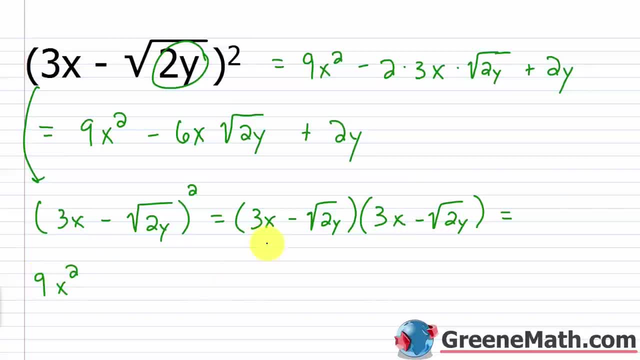 the outer 3x times negative square root of 2y negative 3x times the square root of 2y the inner would be the same thing right? 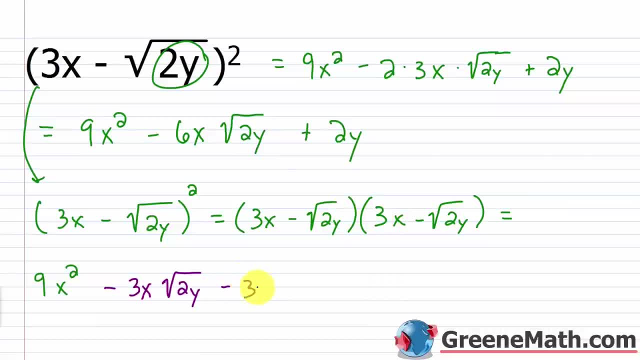 negative square root of 2y times 3x so negative 3x times the square root of 2y and then the last would be negative times negative is positive square root of 2y times square root of 2y is 2y 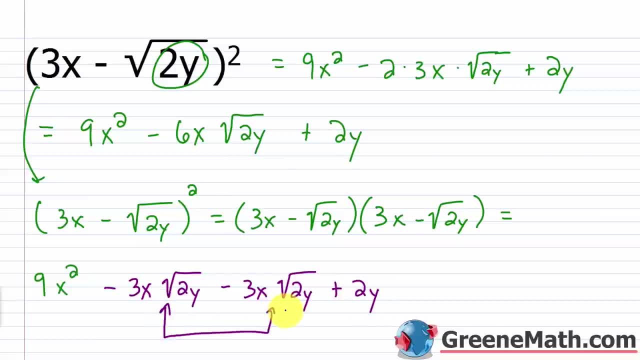 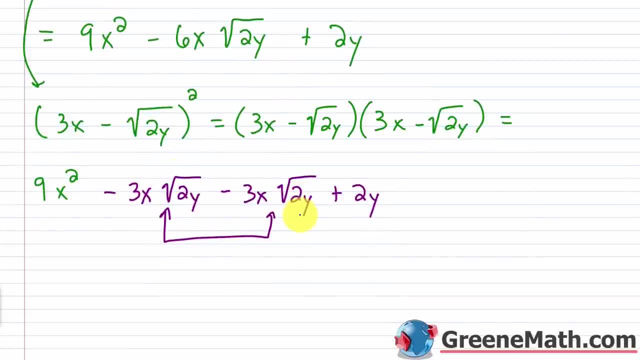 so if I combine the terms in the middle I know that I have like radicals there, so I can do that because I have the same index and the same radicand. I'd have 2y in each case. So really, I just think about negative 3x plus negative 3x, that's negative 6x. So this would end up being 9x squared minus 6x times the square root of 2y and then plus 2y. And again, it's exactly what we got right there. I just used a quicker method when we first did it, and that's the method that you should use, right? Memorize those special 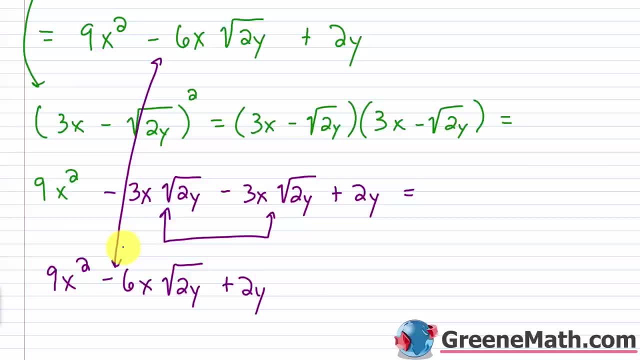 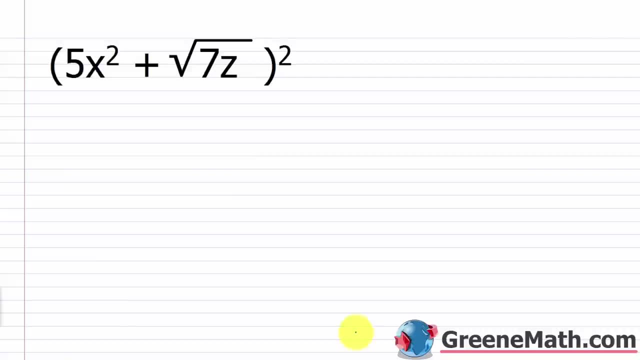 product formulas. And again, they're going to help you for the rest of your life, right? It's just something that's just going to tremendously speed up your processes. All right, let's take a look at another one. And for this one, I'm going to match that formula of the quantity x plus y squared. So this is x squared plus 2xy plus y squared. So exactly what we just looked at, the only difference is going to be your sine, 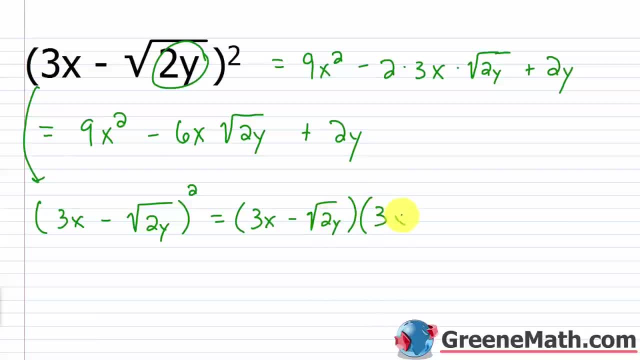 root of 2y times again 3x minus the square root of 2y. So I would just erase this here and show you why. So the first terms 3x times 3x would be 9x squared, The outer 3x times negative square root. 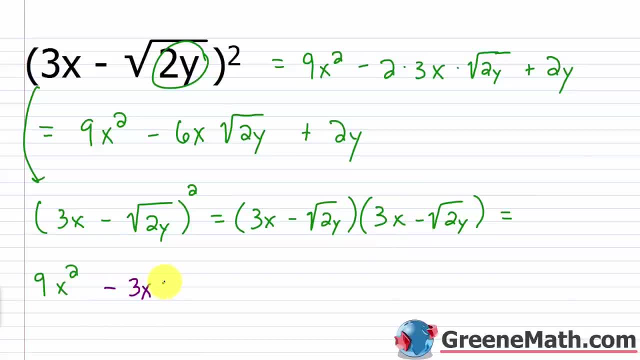 of 2y, negative 3x times the square root of 2y. The inner would be the same thing: right Negative square root of 2y times 3x. So negative 3x times the square root of 2y. And then the last would be: 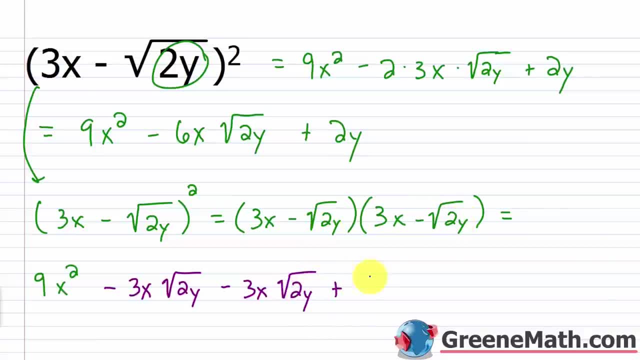 negative times negative is positive. Square root of 2y times square root of 2y is 2y. So if I combine the terms in the middle, I know that I have like radicals there. so I can do that because I have the same index and the same radicand I'd have 2y in each case. 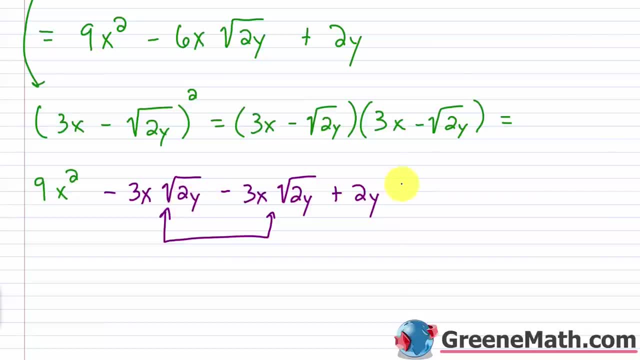 So really I just think about negative 3x plus negative 3x, that's negative 6x. So this would end up being 9x squared minus 6x times the square root of 2y, and then plus 2y. 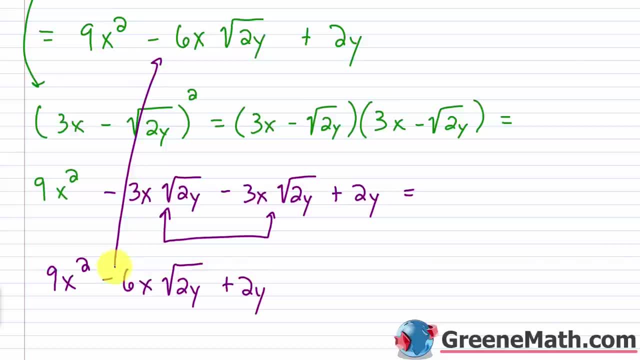 And again, it's exactly what we got right there. I just used a quicker method when we were doing this, We first did it, and that's the method that you should use. right? Memorize those special product formulas And again, they're going to help you for the rest of your life, right? It's just something. 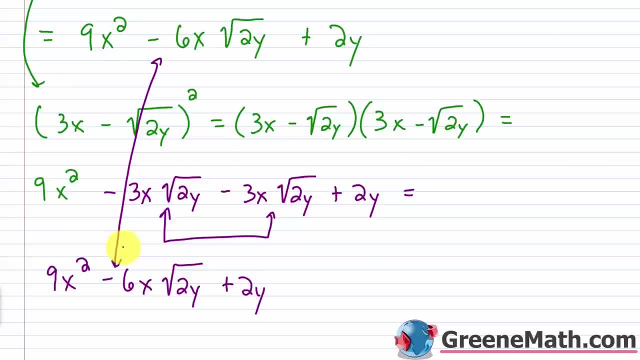 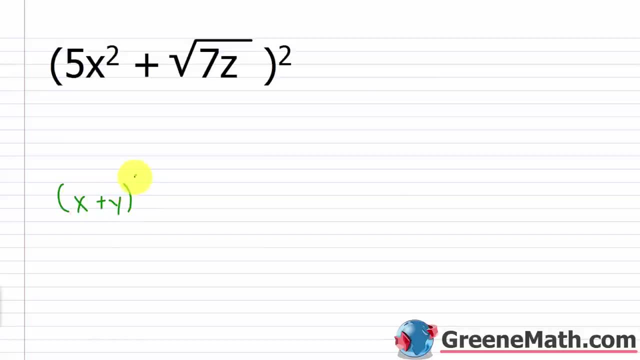 that's just going to tremendously speed up your processes. All right, let's take a look at another one, And for this one I'm going to match that formula of the quantity x plus y squared. So this is x squared plus 2xy plus y squared. So exactly what we just looked at. the only difference is: 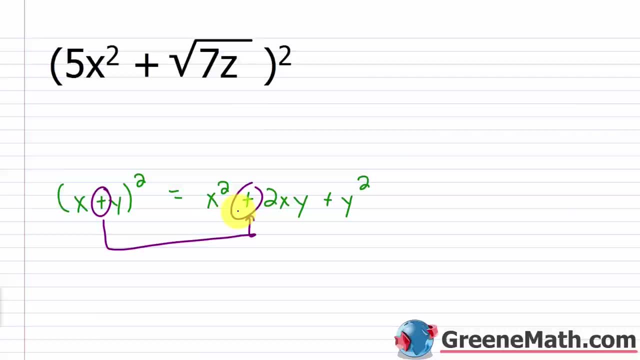 plus, in this case for that second term. right, If I have the quantity x minus y squared, everything is the same, except for that minus sign right there. All the rest is the same. So if I was to do this- and I'm not going to do this one the long way, just to save a little time- 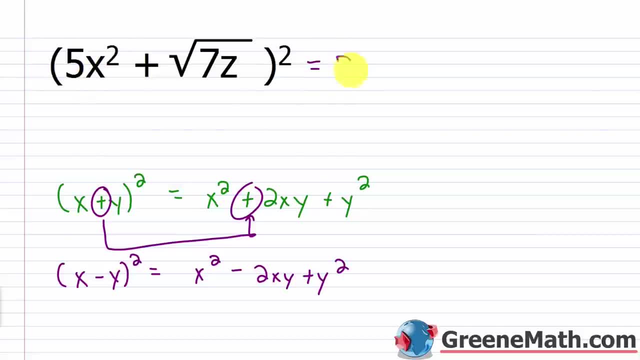 I would say what The first guy squared. So if I square 5, I get 25.. If I square x squared, I get x to the fourth power right. x squared squared, It's the same. Multiply 2 times 2,, that's 4.. Okay, So now the next thing I want to do is I want to. 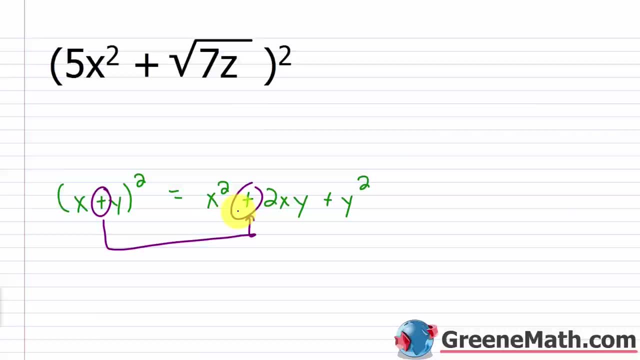 is plus in this case for that second term, right? If I have the quantity x minus y squared, everything is the same except for that minus sign right there. All the rest is the same. So if I was to do this, and I'm not going to do this one the long way, just to save a little time, I would say what? The first guy squared. So if I square 5, I get 25. If I square x squared, I get x to the fourth power, right? x squared squared, keep x the same, multiply 2 times 2, that's 4. Okay. So now the next thing I want to do 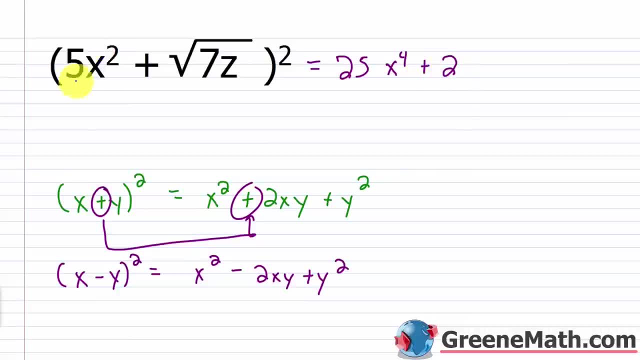 is I want to put plus 2 times this guy right here. So 2 times 5 is 10. Let me just go ahead and write that. So 10 times x squared times this guy, the square root of 7z. And then the last thing I want to do is put plus this guy squared. So if I square the square root of something, I just get the radicand. 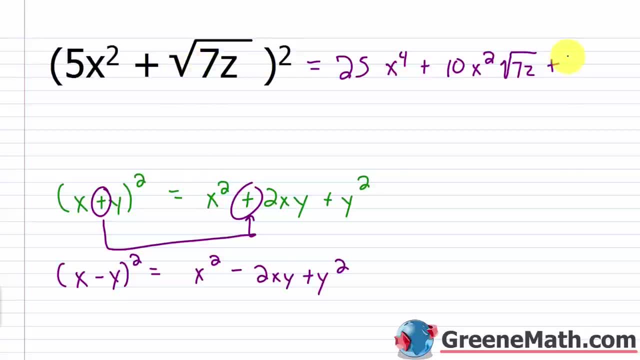 Right? If I square the square root of 7z, I'm just going to get 7z. Now looking at this, there's nothing I can combine here. So my simplified answer would be 25x to the fourth power plus 10x squared times the square root of 7z plus 7z. All right. So now 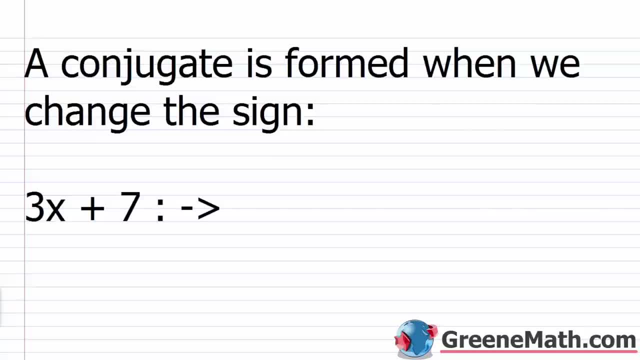 what we're going to talk about for the remainder of this section is what to do when you have a more complex denominator that's involved, and you need to rationalize the denominator, you don't want any radicals in the denominator. But sometimes it's not so simple. You might get something that's more complex. And before we start jumping into that, we have to learn about something known as a conjugate. Okay. So a conjugate is formed when we change the sign of something like this. So if I have 3x plus 7, I would have 3x and I would have 7, but my sine would change. Okay. My sine would change. So the conjugate of 3x plus 7 is just 3x 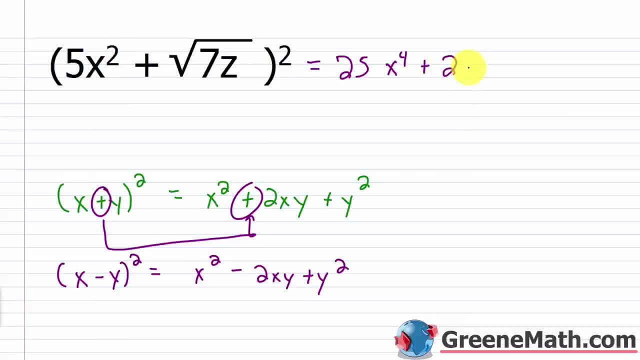 put plus 2 times this guy right here. So 2 times 5 is 10.. Let me just go ahead and write that. So 10 times x, squared times this guy, the square root of 7z. And then the last thing I want to do is put: 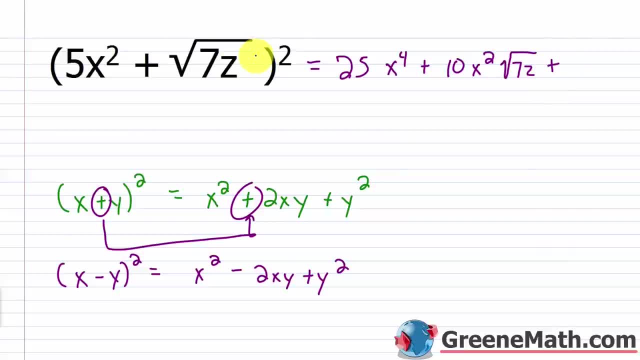 plus this guy squared. So if I square the square root of something, I just get the radicand back. if I square the square root of 7z, I'm just going to get 7z. Now, looking at this, there's nothing I can combine here. So my simplified answer would be: 25x to the fourth. 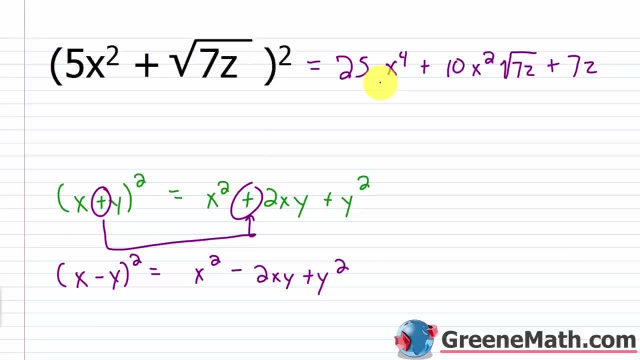 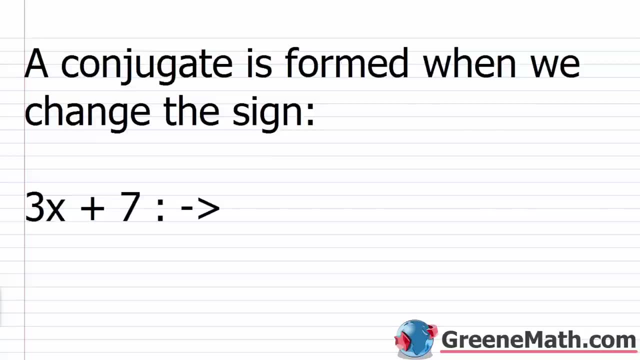 power plus 10x squared times the square root of 7z plus 7z. All right, So now what we're going to talk about for the remainder of this section is what to do when you have a more complex denominator that's involved and you need to rationalize the denominator, right, You don't? 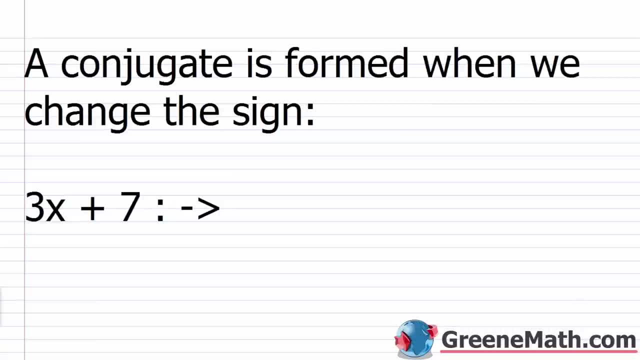 have to write the radicals in the denominator, but sometimes it's not so simple. You might get something that's more complex, And before we start jumping into that, we have to learn about something known as a conjugate. Okay, So a conjugate is formed when we change the sign. 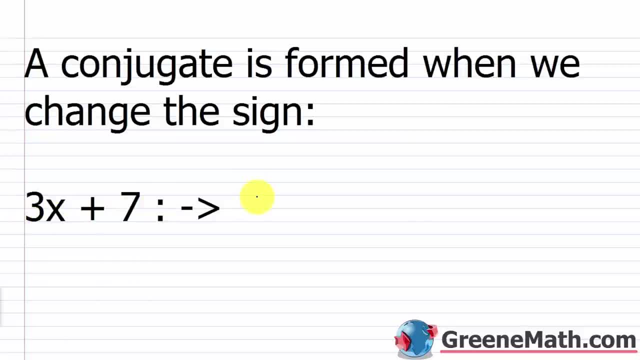 of something like this: So if I have 3x plus 7, I would have 3x and I would have 7, but my sign would change. Okay, My sign would change. So the conjugate of 3x plus 7 is just. 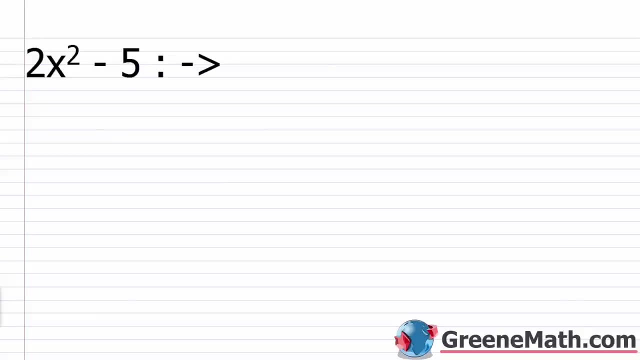 3x minus 7.. Another example: if I had something like 2x squared minus 5, the conjugate would be change the sign so 2x squared. this would become plus, and then this would stay the same. So the 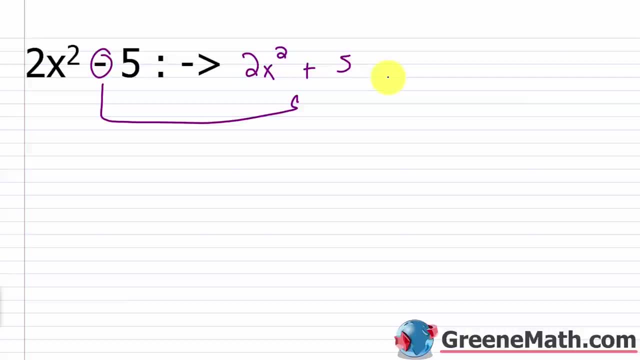 terms are the same, I'm just changing the sign. So if I had, let's say, x plus y as an example, the conjugate would be x minus y. If I saw a plus b, the conjugate would be a minus b. 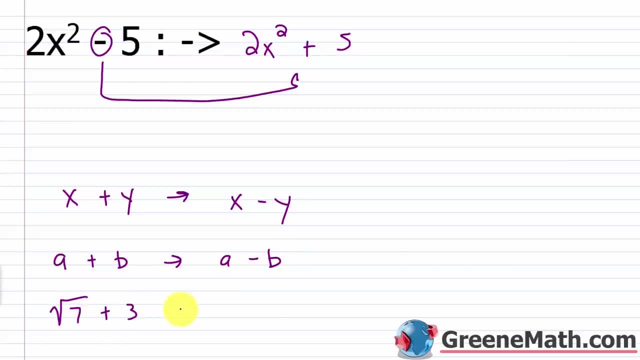 If I saw the square root of 7, plus 3,, the conjugate would be square root of 7 minus 3.. I'm keeping the two terms the same. All I'm doing is just changing the sign. right, It's very, very simple. All right. So now that. 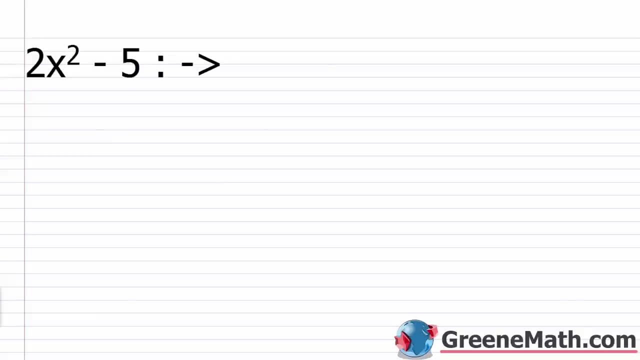 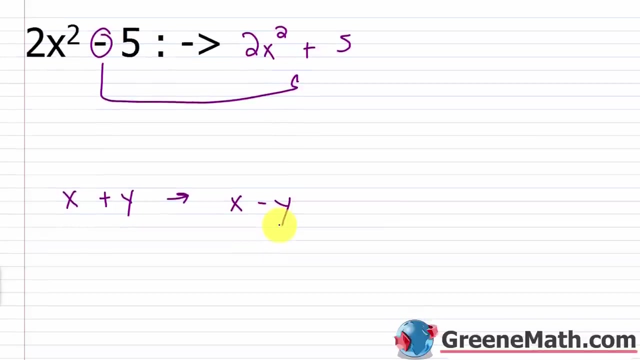 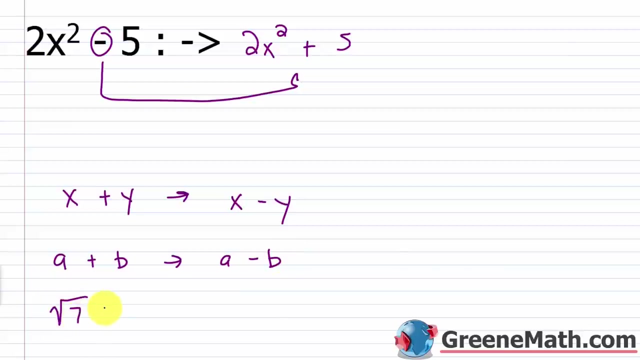 minus 7. As another example if I had something like 2x squared minus 5 the conjugate would be change the sign so 2x squared this would become plus and then this would stay the same. So the terms are the same I'm just changing the sign. So if I had let's say x plus y as an example the conjugate would be x minus y. If I saw a plus b the conjugate would be a minus b. If I saw the square root of 7 plus 3 the conjugate would be square root of 7 minus 3. I'm keeping the two 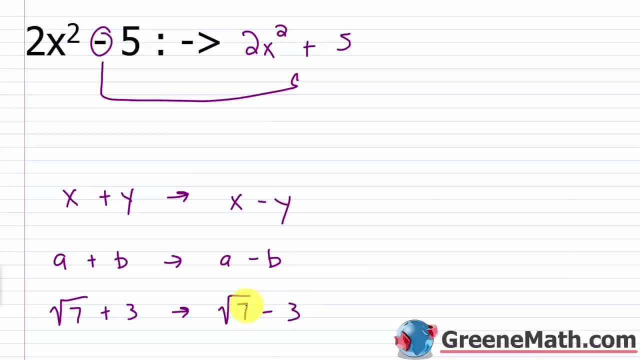 terms the same all I'm doing is just changing the sign. It's very very simple. All right so now that 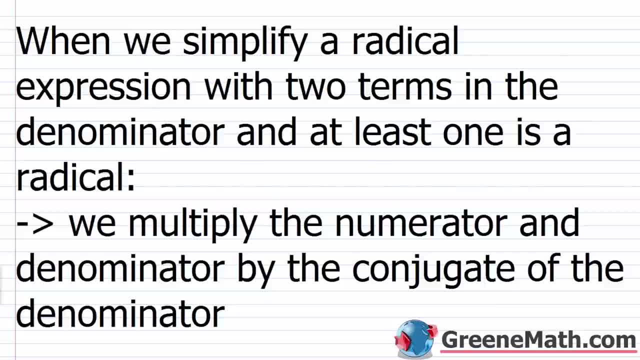 we know what a conjugate is let me just read this to you. So when we simplify a radical expression with two terms in the denominator and at least one is a radical remember you can't have any radicals in your denominator what you're going to do to get that radical out of the denominator we're going to multiply the numerator and denominator by the conjugate of the denominator. Okay and the reason that's going to 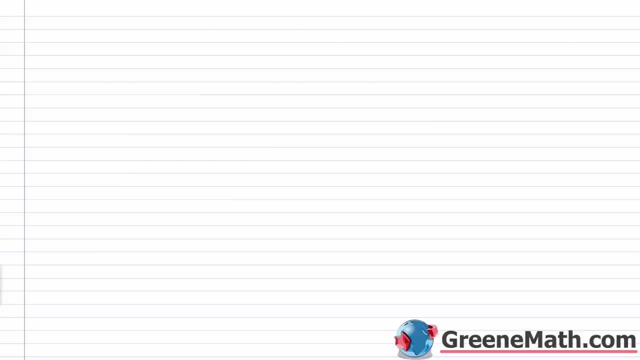 work is you're setting up a scenario of something like this a plus b that quantity times a minus b. Okay you have the same term okay in the first position of each you have the same terms in the second position of each your difference is the sign. So what's going to happen is the middle two terms when you do foil there drop out you know we saw this earlier in the lesson where we talked about you know our special products formulas this ends up being what a squared the first guy squared minus b squared right the second guy squared. Very very easy to kind of calculate that the two terms from the middle are going to drop out and you're going to add up the two terms and you're going to add up the two terms and you're going to add up the two terms and you're going to end up with a denominator that 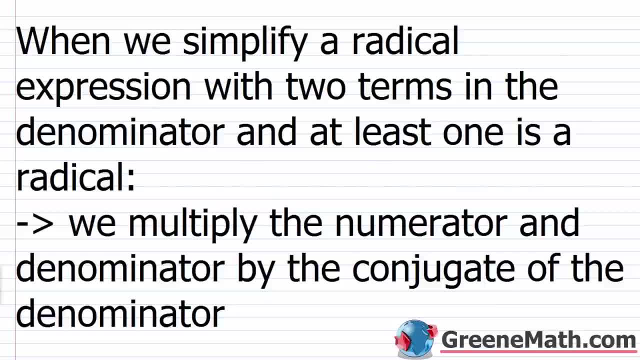 we know what a conjugate is. let me just read this to you. So when we simplify a radical expression with two terms in the denominator and at least one is a radical, remember you can't have any radicals in your denominator. what you're going to do to get that radical out of the denominator? 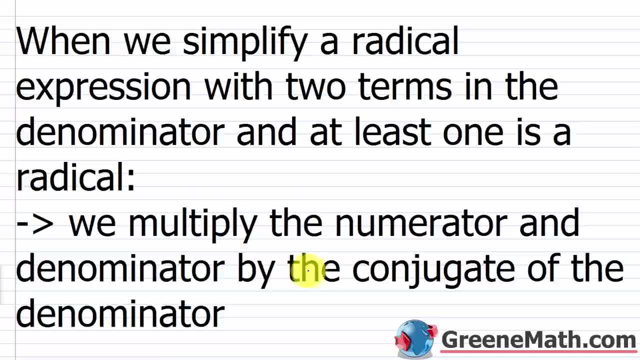 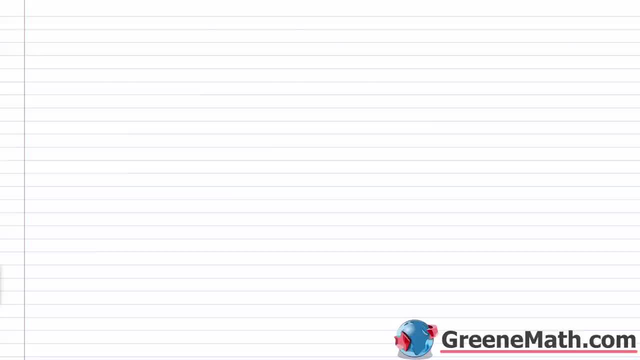 we're going to multiply it by the denominator. So we're going to multiply it by the denominator. multiply the numerator and denominator by the conjugate of the denominator. And the reason that's going to work is you're setting up a scenario of something like this: a plus b. 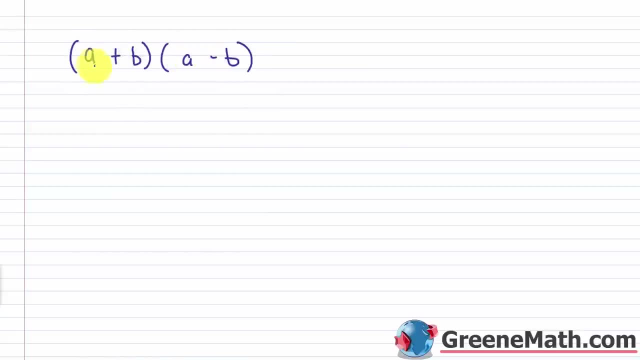 that quantity times a minus b. You have the same terms in the first position of each. You have the same terms in the second position of each. Your difference is the sign. So what's going to happen is the middle two terms. when you do FOIL there, drop out. you know, we saw this earlier in the 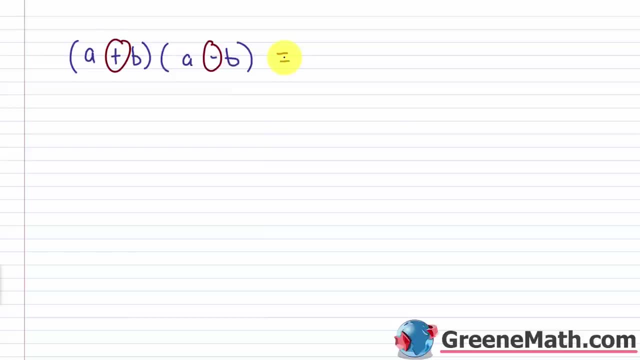 lesson where we talked about, you know, our special products formulas. This ends up being what: a squared, the first guy squared, minus b squared right, The second guy squared, Very, very easy to kind of calculate that The two terms from the middle are going to drop out. 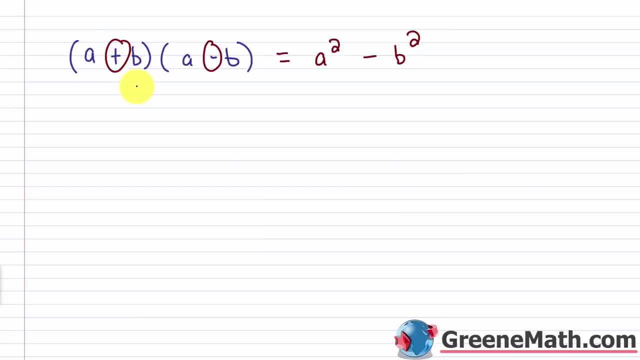 and you're going to end up with a denominator that is radical free. So let's see an example. So we'll start out with this kind of easy one. We have 8 over 6 minus the square root of 5.. So I'd multiply this by the conjugate of the denominator. right? We're going to do that to. 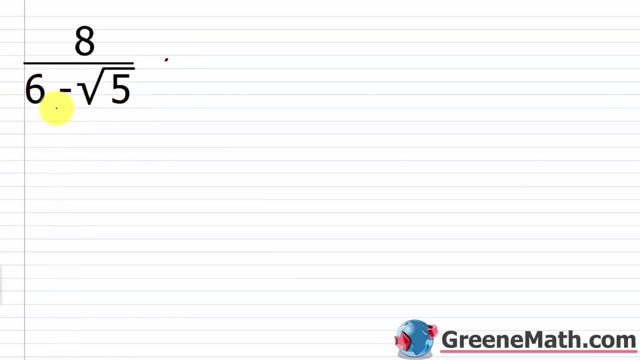 the numerator and denominator. So if I think about the conjugate, it's 1.. Keep the terms the same, So 6 and square root of 5, 6 and square root of 5.. But the sign is going to change right, So instead. 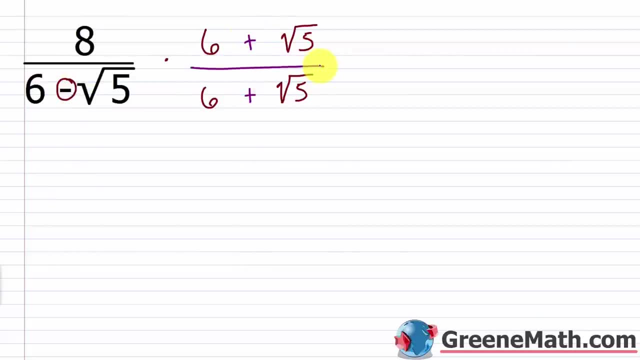 of a minus, it's going to be a plus. Now, am I doing anything illegal if I'm multiplying this by this? No, This is a complex form of 1, right, 6 plus square root of 5, 6 plus square root of 5,. 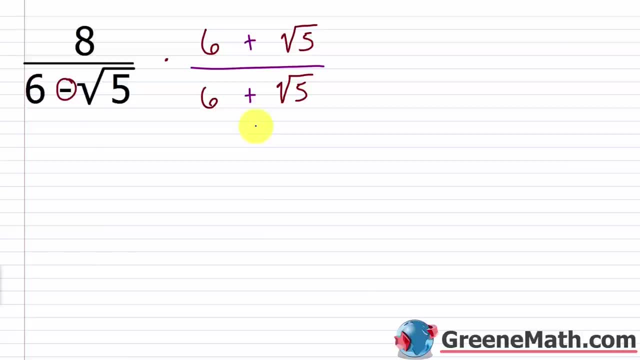 square root of 5 over 6 plus square root of 5, complex form of 1.. I multiply by 1, and I don't change the value right, So this is legal. Now in the numerator, if I multiply, I just use my. 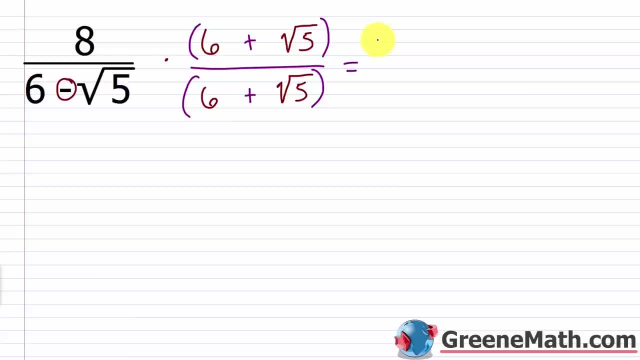 distributive property, right? So I'm just going to say: well, 8 times 6 is 48. Then plus 8 times square root of 5 is just 8 times square root of 5.. That's simple enough, right? I can't do anything. 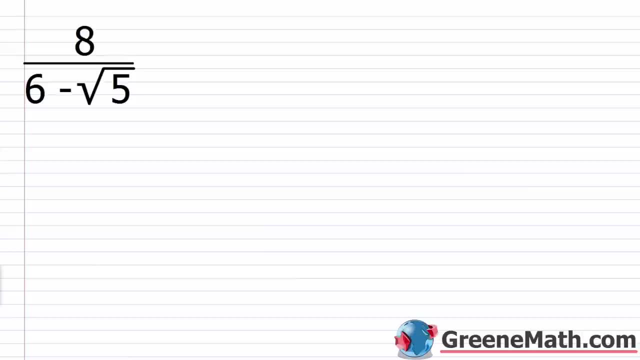 is radical free. So let's see an example so we'll start out with this kind of easy one we have eight over six minus the square root of five so I'd multiply this by the conjugate of the denominator all right we're going to do that to the numerator and denominator so if I think about the conjugate it's one keep the terms the same so six and square root of five six and square root of five but the sign is going to change right so instead of a minus it's going to be a plus now am I doing anything illegal if I'm multiplying this by this no this is a complex form of one right six plus square root of five over six plus square root of five complex form of one I multiply by one I don't change the value right so this is legal now in the numerator if I multiply I just use my distributive property right so I'm just going to say well eight times six is 48 then plus eight times square root of five is just eight times square root of five that's simple enough. 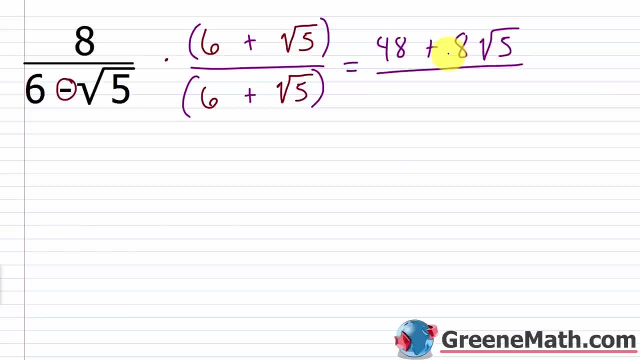 All right I can't I can't do anything else there and then for the denominator again realize that you have that pattern where you have six and six same term square root of five square root of five same term different signs negative positive okay so I can use that little formula to speed up the process and just say okay we'll have the first guy squared six squared is 36 minus the second guy squared square root of five squared is just five so my denominator is going to be 31 so I would have 48 plus 8 times square root of 5 over 36 minus 5 is 31. So my denominator now is radical free and again that's our goal here because if we report our answer with a radical in the denominator we're going to get points taken away at minimum right it's not considered simplified. All right let's look at one that's a little bit harder. Let's look at one that's not considered simplified. 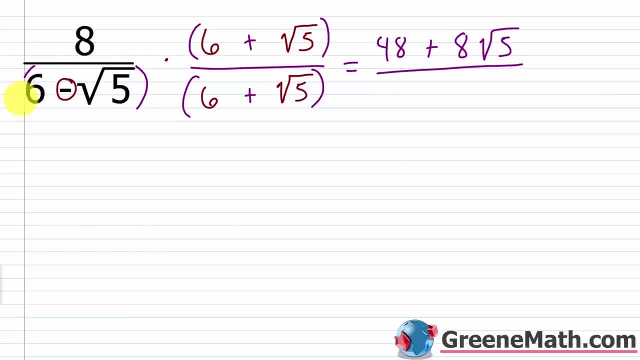 else there. And then for the denominator again, realize that you have that pattern where you have 6, and 6, same term, square root of 5, square root of 5, same term. different signs: negative, positive. okay, So I can use that little formula to speed up the process and just say, okay. 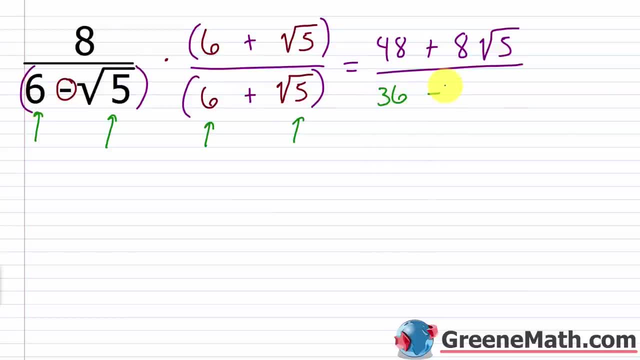 we'll have the first guy squared 6 squared is 36, minus the second guy squared Square root of 5 squared is just 5.. So my denominator is going to be 31.. So I would have 48 plus 8 times square root. 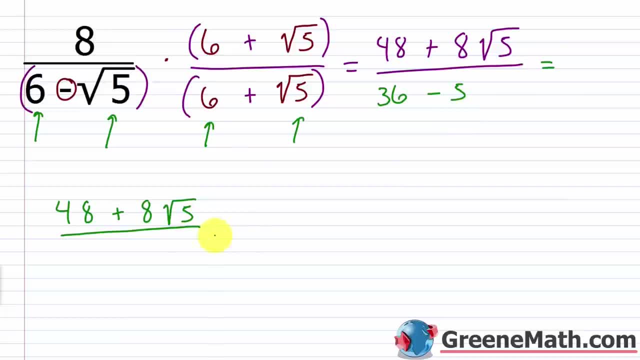 of 5 over 36 minus 5 is 31.. So my denominator now is radical free. And again, that's our goal here, because if we report our answer with a radical in the denominator, we're going to get points taken away at minimum. right, It's not considered simplified. All right, let's look at one that's: 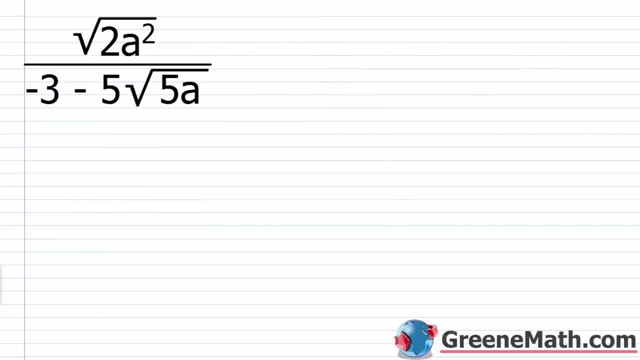 a little bit harder- Not harder, but more tedious. We have the square root of 2a squared over negative 3 minus 5 times square root of 5a. So the first thing I do is, if I see something that's I can simplify, I just do it right. This really should be what This is: a squared underneath a. 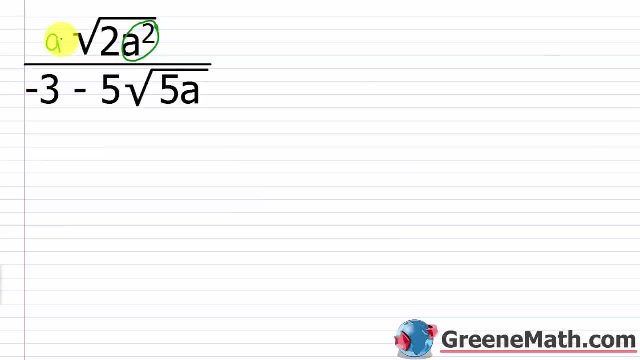 square root, So this would be a times the square root of 2.. So I should really just line this out and write it like that, right? And I can let me kind of just write it over here as a times square root of 2 over negative 3 minus 5 times square root of 5a. So let me just kind of move this down. 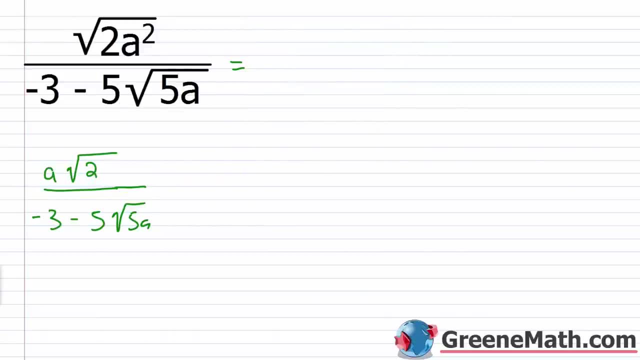 here to get us some more room Again, if I want to remove the radical from the denominator, in this case I'm going to multiply the numerator and denominator by the conjugate of that denominator. So to get my conjugate the terms stay the same. So I'd have negative 3 and I'd have 5 times square root. 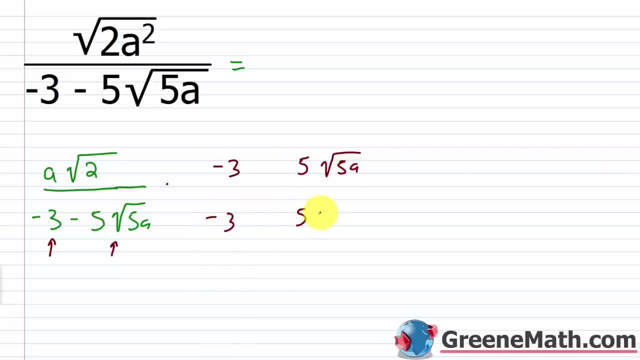 of 5a. That stays the same. So let's do that in each case. What's going to change as a sign? So in this case it's negative. So this would be positive and this would be positive, Okay, so. 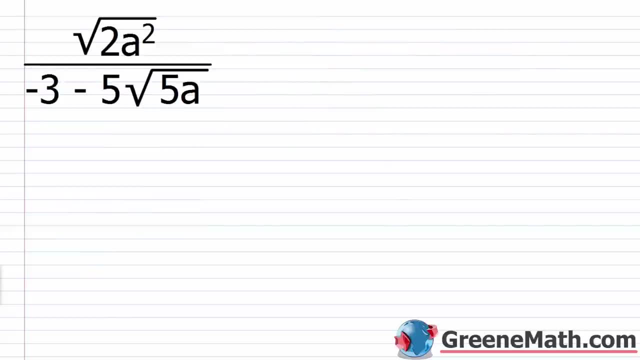 little bit harder not harder but more tedious we have the square root of 2a squared over negative 3 minus 5 times square root of 5a so the first thing I do is if I see something I can simplify just do it right this this really should be one this is a squared underneath a square root so this would be a times the square root of two so I should really just line this out and write it like that right and I can let me kind of just write it over here as a square root of two so I'm gonna write I'm gonna multiply this so I can get negative three times square root of two over negative three minus five times square root of 5a so let me just kind of move this down here to get us some more room again if I want to remove the radical from the denominator in this case I'm going to multiply the numerator and denominator by the conjugate of that denominator so to get my conjugate the terms stay the same so I'd have negative three what's going to change as a sign so in this case it's negative so this would be positive and this would be positive okay so now that we've worked that out a times square root of 2 times negative 3 is what this is negative 3a times the square root of 2 can't do anything else with that then plus i've got 5 times a that's 5a times the square root of 2 times the square root of 5a 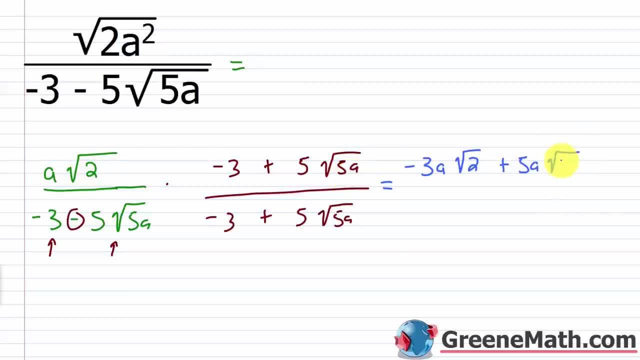 so i'm going to write that as the square root of 5 times 2 or 10 times a so the numerator nothing else i can do there it's just going to stay as negative 3a times square root of 2 plus 5a times square root of 10a okay what about my denominator what can i do here well again we're going to use that formula i've got the same term here and here same term here and here signs are different right so square the first guy square negative 3 you get 9 then minus square the second guy 5 squared is 25 and then the square root of 5a squared would be 5a so you get 25 times 5 or 125 and then a now can i simplify that any further no these are not like terms right 9 is not a like term with negative 125a can't do anything further so my simplified answer here is negative 3a times the square root of 2 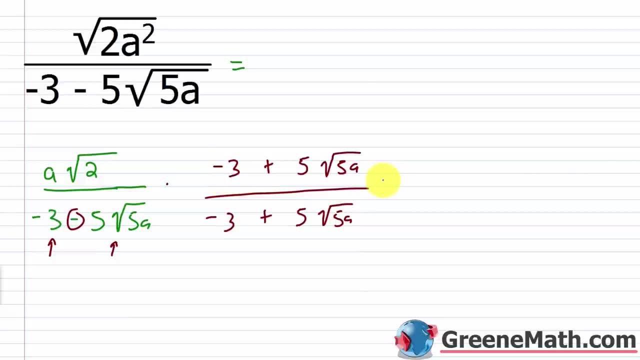 now that we've worked that out, we're going to do the next thing. We're going to do the next thing: A times square root of 2, times negative 3 is what This is negative 3a times the square root of 2.. Can't do anything else with that. Then, plus, I've got 5 times a. 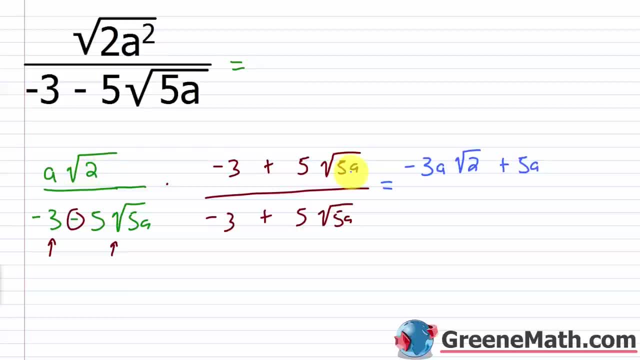 That's 5a Times the square root of 2 times the square root of 5a. So I'm going to write that as the square root of 5 times 2, or 10, times a. So the numerator nothing else I can do there. It's just going to stay as negative 3a times square root of 2, plus negative 2.. So I'm just going to copy that in just me, or down. I could change the numerator until I get the denominator. So I'm going to get rid of the denominator and 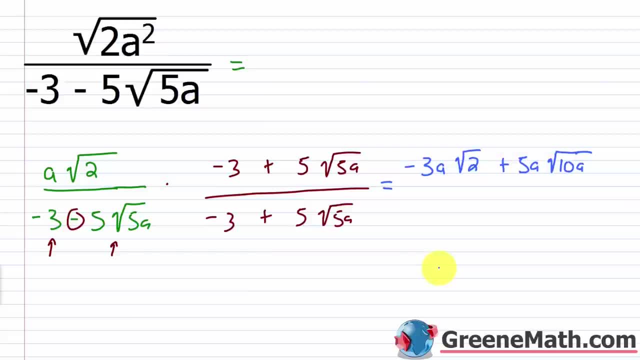 then I'm just going toれて the numerator in the numerator, or plus or less than that: 3a times square root of 2 plus 5a times square root of 10a. Okay, what about my denominator? What can I do here? Well, again, we're going to use that formula. I've got the same term here. 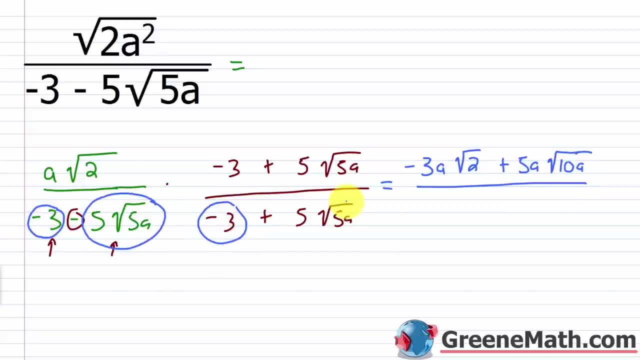 and here same term. here and here Signs are different, right, So square the first guy, square negative 3, you get 9.. Then minus square the second guy, 5 squared is 25.. And then the square root of 5a squared would be 5a. So you get 25 times 5, or 125. 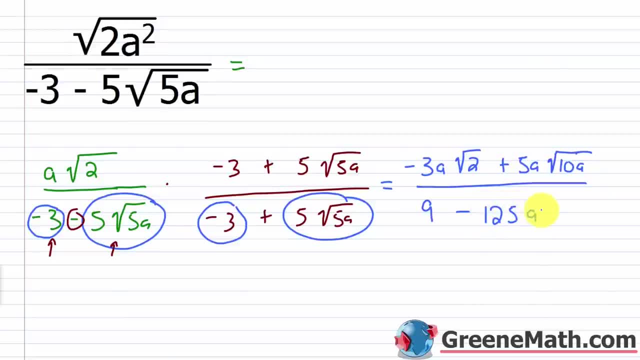 and then a. Now can I simplify that any further? No, These are not like terms, right? 9 is not a like term with negative 125a. Can't do anything further. So my simplified answer here is: negative 3a times the square root of 2 plus 5a times the square root of 10a over 9 minus 125a. 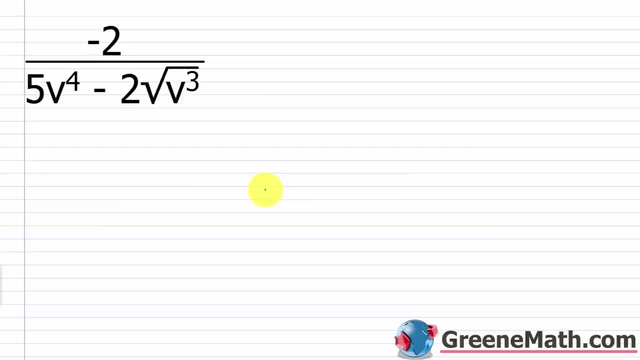 All right, for the next one. I have negative 2 over 5v to the fourth power minus 2 times the square root of v cubed. Now what I can do before I even start. I can simplify, So negative 2 over. 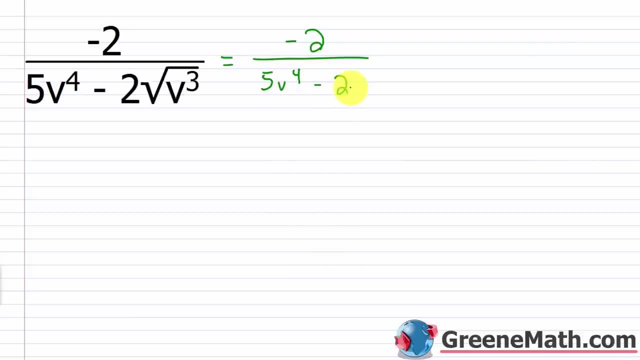 5v to the fourth power minus 2.. The square root of v cubed. I can think about the square root of v cubed as the square root of v squared times. the square root of v Square root of v squared is v. 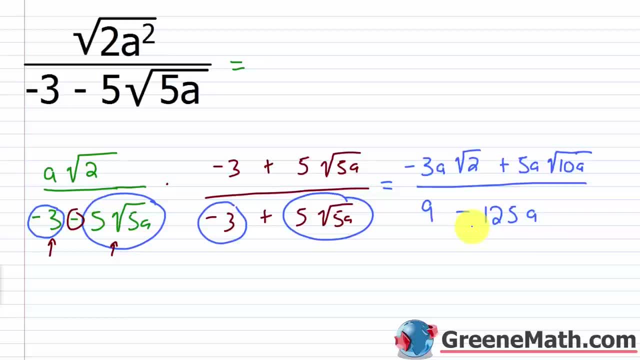 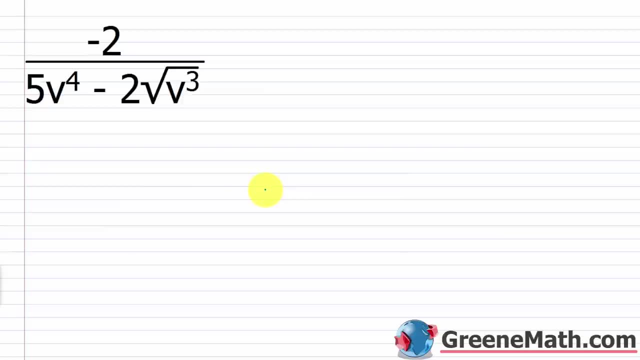 plus 5a times the square root of 10a over 9 minus 125a all right for the next one i have negative 2 over 5v to the fourth power minus 2 times the square root of v cubed now what i can do before i even start i can simplify so negative 2 over 5v to the fourth power minus 2 the square root of v cubed i can think about the square root of v cubed as the square root of v squared times the square root of v squared of v squared is v so i can write this as minus 2v times the square 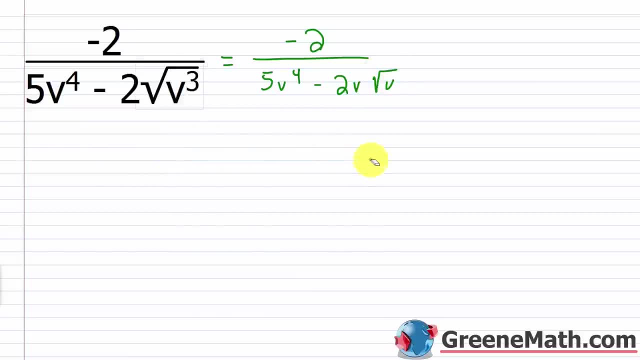 root of v so i like to simplify before i even think about anything else because it just makes my calculations easier in the end so let me kind of drag this down so we have a little room to work okay let me put this over here and so now i want to multiply the numerator and denominator 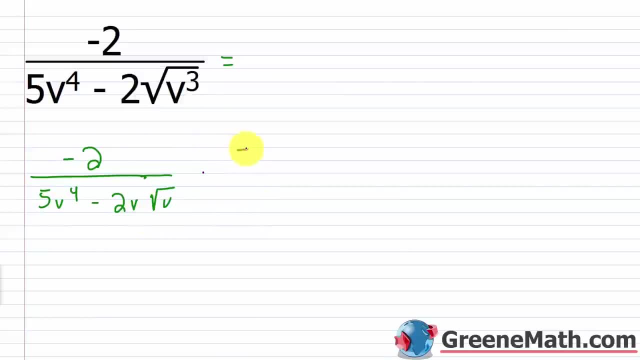 by the conjugate of the denominator so the terms are the same 5v to the fourth power and 2v times square root of v over we have 5v to the fourth power and 2v times square root of v the signs are going to be different right so this is a negative this will be plus and plus all right so in the numerator let's start out negative 2 times 5 is negative 10 so that's negative 10 and then we have v to the fourth power then negative 2 times 2 would be negative 4 and then times v and then times the square root of v then over 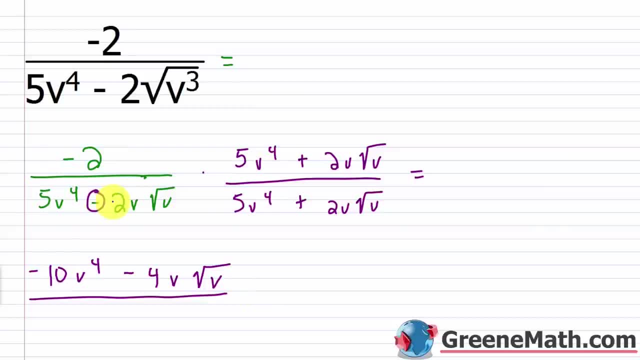 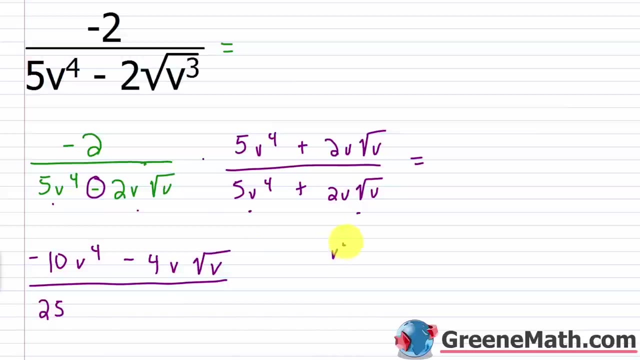 now again if i'm using that formula i don't need to go through and do foil right i have the same thing here and here same thing here and here the signs are different so the first guy squared 5v to the fourth power squared 5 squared we know is 25 v to the fourth power squared so v to the fourth power squared v stays the same 4 times 2 is 8 then minus the next guy is going to be squared so 2v squared is what that's 4v squared square root of v squared is v so i'd have v squared times 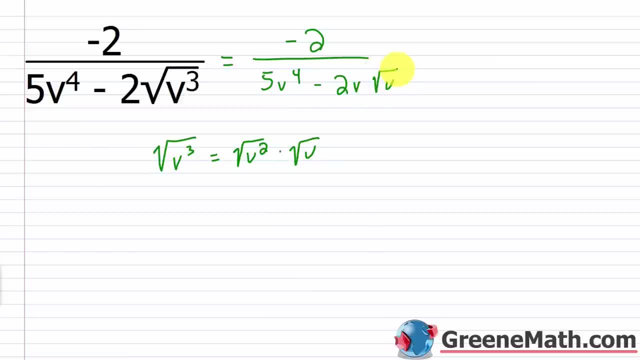 So I can write this as minus 2.. 2v times the square root of v. So I like to simplify before I even think about anything else, because it just makes my calculations easier in the end. So let me kind of drag this down. so we. 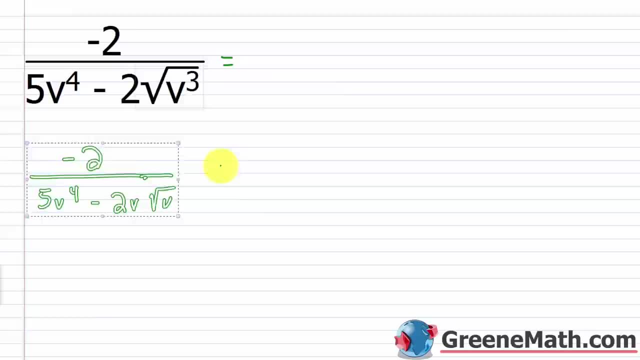 have a little room to work. Okay, let me put this over here. And so now I want to multiply the numerator and denominator by the conjugate of the denominator. So the terms are the same: 5v to the fourth power and 2v times square root of v. over we have 5v to the fourth power and 2v. 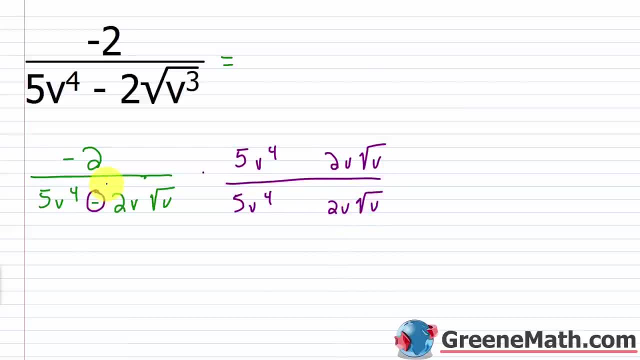 times square root of v, The signs are going to be different, right? So this is a negative. This will be plus and plus, All right, So in the numerator let's start out: Negative 2 times 5 is negative 10.. So that's negative 10.. And then we have v to the fourth power. 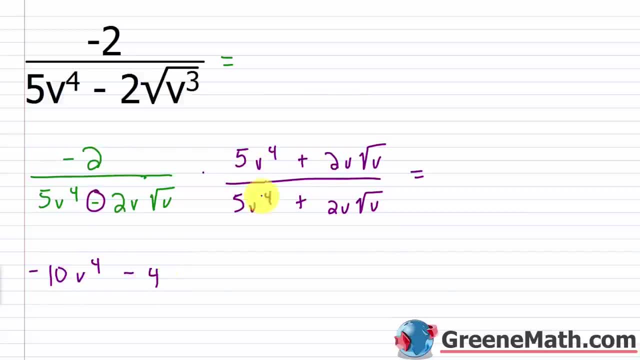 Then negative 2 times 2 would be negative 4.. And then times v And then times the square root of v, Then over Now again, if I'm using that formula, I don't need to go through and do FOIL, right I? 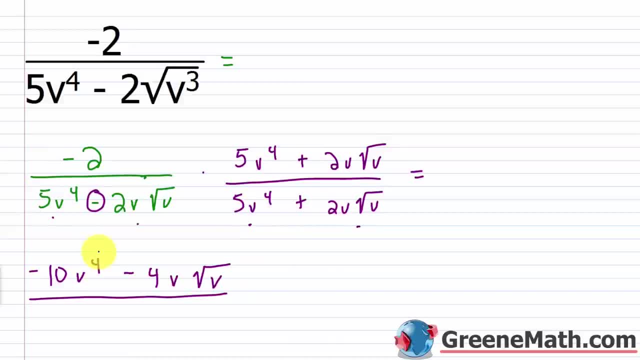 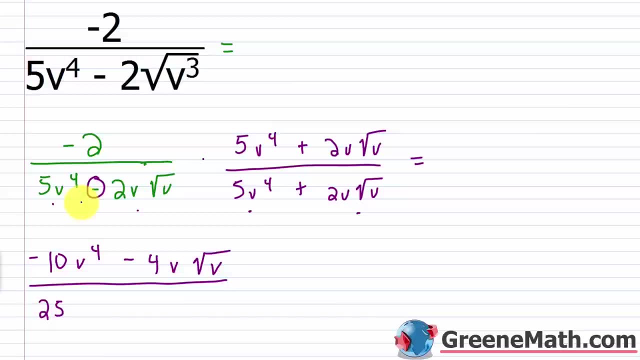 don't need to go through and do FOIL The same thing here and here, Same thing here and here. The signs are different. So the first guy squared 5v to the fourth power squared. 5 squared, we know, is 25.. v to the fourth power squared, So v to the fourth power squared. v stays the same 4 times. 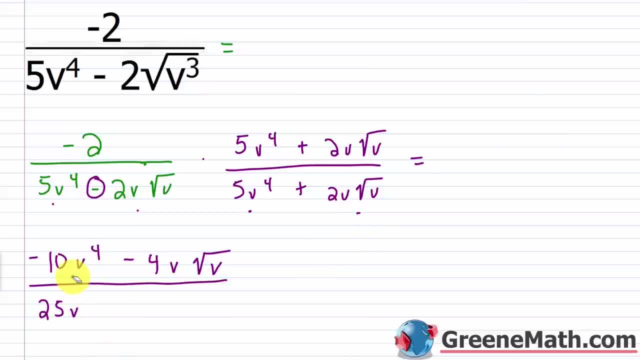 2 is 8.. Then minus The next guy is going to be squared. So 2v squared is what That's: 4v squared. Square root of v. Square root of v squared is v. So I'd have v squared times v, or v cubed, v cubed. So now my 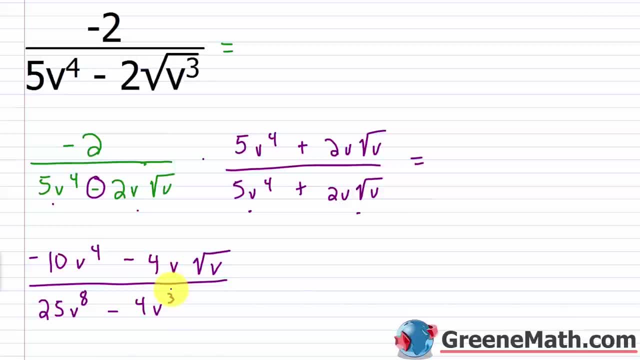 answer here: negative 10v to the fourth power minus 4v times the square root of v over 25v to the eighth power minus 4v cubed. So is there anything else I can do to simplify here? Well, yes, there is Notice that you have that variable v here, here, here and here. So that means I. 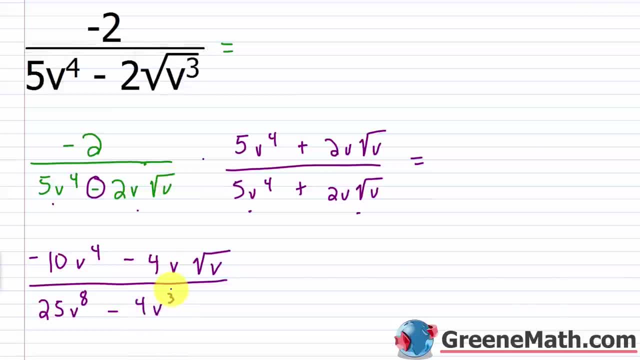 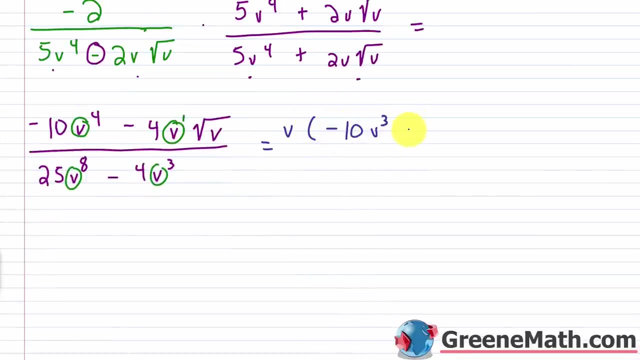 v or v cubed v cubed so now my answer here negative 10 v to the fourth power minus 4v times the square root of v over 25 v to the eighth power minus 4v cubed so is there anything else i can do to simplify here yes there is notice that you have that variable v here here here and here so that means i could factor a v out from the numerator and the denominator and i could cancel now you're going to only be able to think about the lowest exponent on any of them in this case that's going to be a 1 right so if i factored out a v from the numerator let me kind of scroll down get a little room going i would have inside of parentheses negative 10 times v cubed minus from here i'd have a 4 the v is getting factored out so that's gone it's just v to the first power so that's gone times square root of v and then over for this guy if i factor out a v i'll have 25v to the seventh power minus 4v squared now i can cancel this v with this v and now my simplified answer is going to be negative 10 v cubed minus 4 times square root of v over 25 v to the seventh power minus 4v cubed 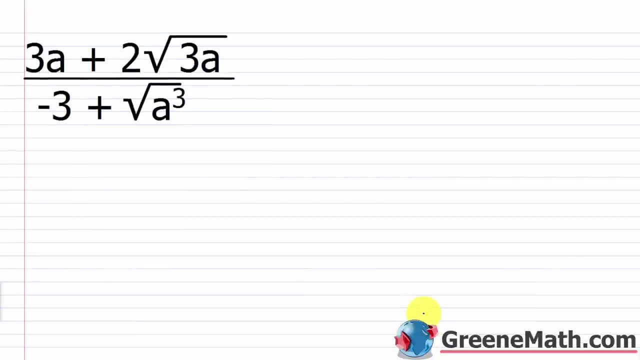 squared. All right, for the last problem we're going to look at, I have 3a plus 2 times square root of 3a over negative 3 plus square root of a cubed. So again, if there's something I can 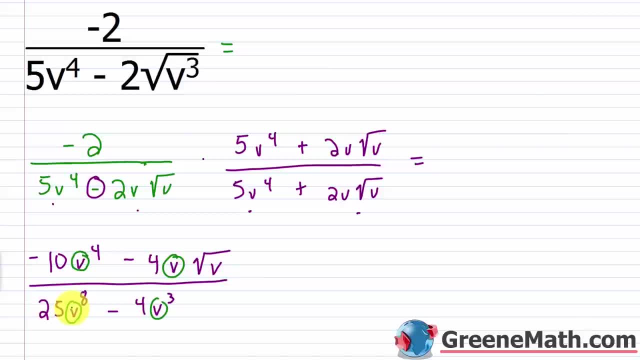 could factor a v out from the numerator and the denominator And I could cancel. Now you're going to only be able to think about the lowest exponent on any of them. In this case, that's going to be a 1, right? So if I factored out a, 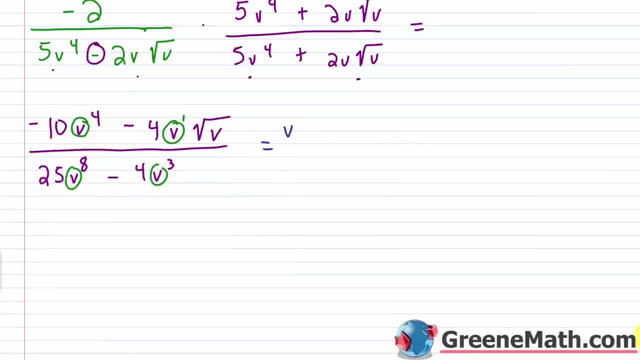 v from the numerator. let me kind of scroll down. get a little room going. I would have inside of parentheses negative 10 times v. cubed minus from here I'd have a 4.. The v is getting factored out, So that's gone. It's just v to the first power, So that's gone. Times: square root of v And then. 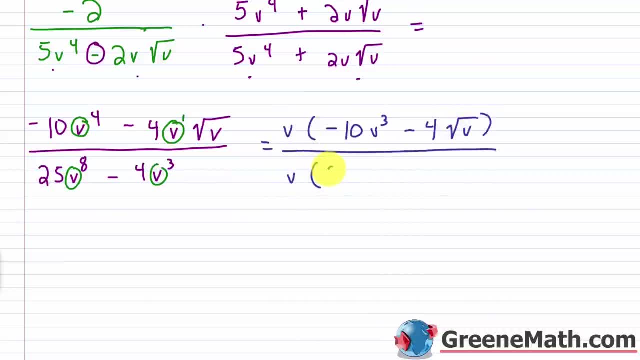 over This guy. if I factor out a v, I'll have 25v to the seventh power minus 4v squared. Now I can cancel this v with this v. And now my simplified answer is going to be negative 10v. 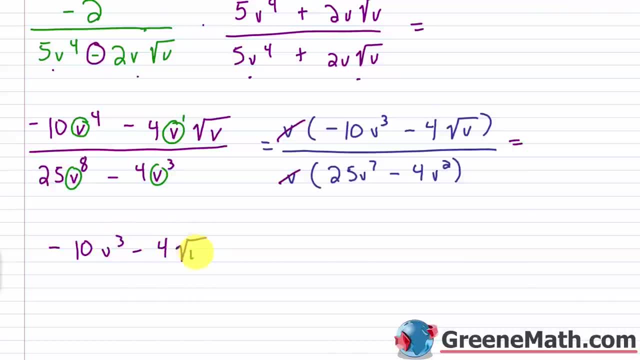 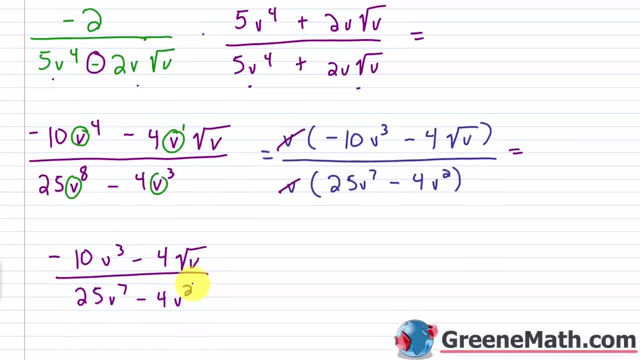 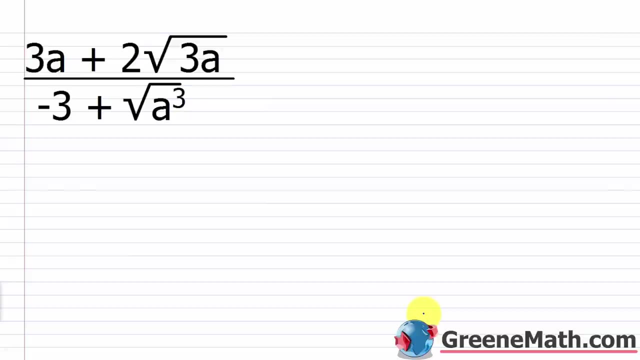 cubed minus 4 times square root of v over 25v to the seventh power minus 4v squared. All right, For the last problem we're going to look at. I have 3a plus 2 times square root of a over negative 3 plus square root of a cubed. So again, if there's something I can simplify before, 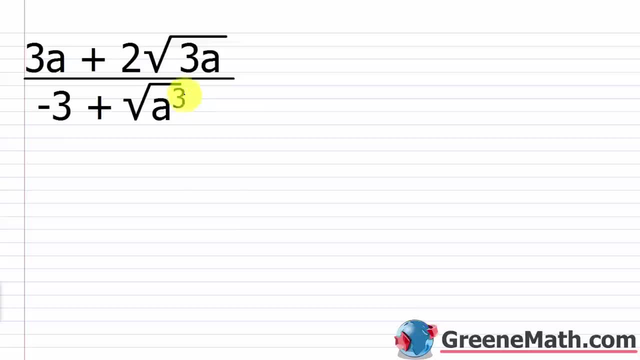 I start, I want to go ahead and do that. I know that this right here. if I have the square root of a cubed, really that's a times square root of a right. Think about the square root of a cubed. 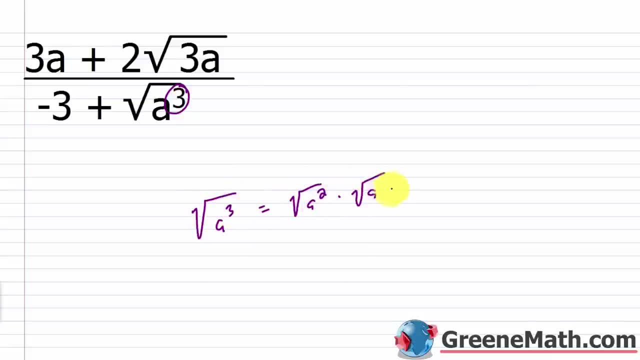 as square root of a squared times square root of a. This is really a, So it's a times square root of a. So let's, let's just simplify this as 3a plus 2 times the square root of 3a over negative 3 plus a times the square root of a. Let's drag this down here to: 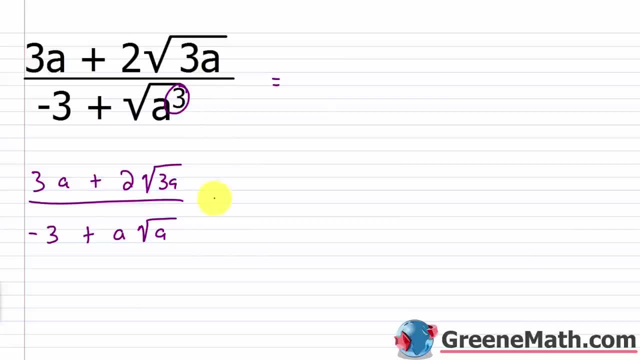 get a little room going And we're going to multiply the numerator and denominator by the conjugate of the denominator. So at this point we know that would be negative 3 minus right. We're changing the sign a times the square root of a, So negative 3 minus a times square root of a. 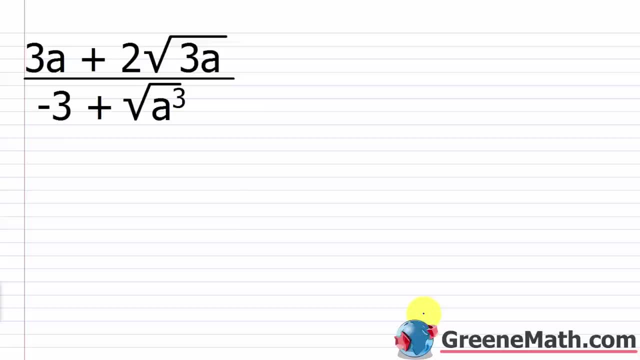 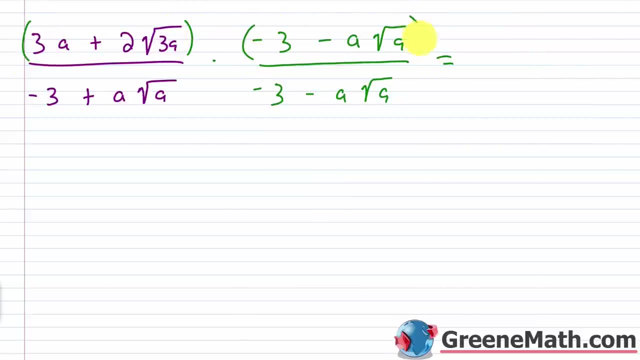 simplify before I start, I want to go ahead and do that. I know that this right here, if I have the square root of a cubed, really that's a times square root of a, right? Think about the square root of a cubed as square root of a squared times square root of a. This is really a, so it's a times square root of a. So let's just simplify this as 3a plus 2 times the square root of 3a over negative 3 plus a times the square root of a. Let's drag this down here to get a little room going. And we're going to multiply the numerator and denominator by the conjugate of the denominator. So at this point we know that would be negative 3 minus, right, we're changing the sign, a times the square root of a cubed. So we're going to multiply the numerator and denominator by the square root of a. So negative 3 minus a times square root of a. All right, so now that we've got that figured out, let's multiply. So for the numerator here, I'm going to use foil. It's going to make it easy. 3a times negative 3 is negative 9a. For the outer, I've got 3a times negative a times square root of a. So that's going to be negative. 3a times a is 3a squared, and then times square root of a. For the inner, I've got 2 times square root of a cubed. So that's going to be square root of 3a times negative 3. So that's negative 6 times square root of 3a. And then for the last, I'm going to have 2 times negative a, or negative 2a, times the square root of 3a times 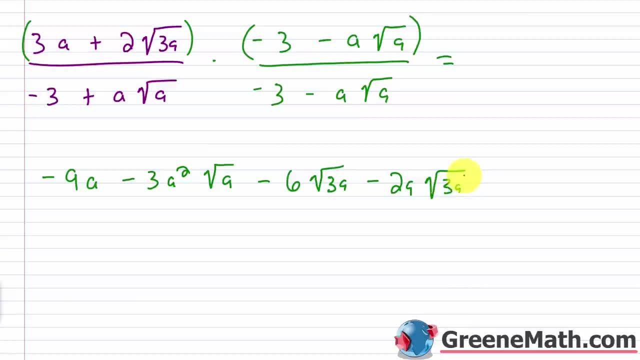 the square root of a. So that would be the square root of 3a squared. So I know the square root of a squared is a. So I can pull that out and make this a squared times the square root of 3. Now, is there anything I can do to simplify here? 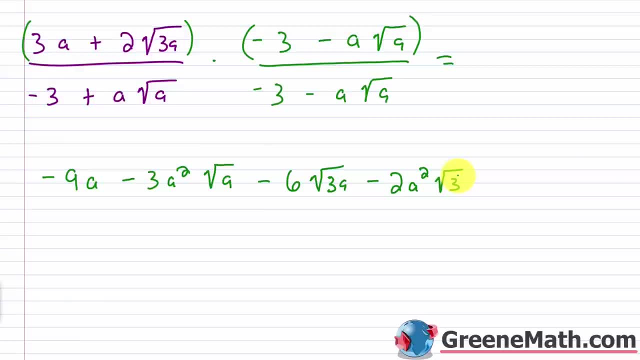 No, there's not. There's nothing else I can do. I know it's long, but there's nothing I can do to simplify. So then this is over. Now, I'm going to use my special products formula here. And that tells me to take the first guy and square it. Negative 3 squared is 9. And then minus the second guy squared. So then that would be a squared times square root of a times square root of a would be a. So really, a squared times a, or a cubed. So my denominator becomes 9 minus a cubed. And then I'm going to take the first guy and square it. And then I'm going to take the 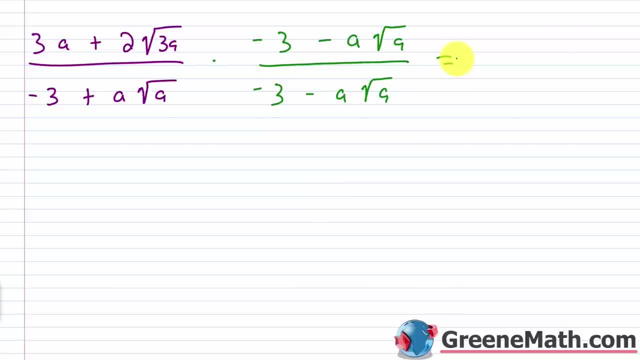 All right. So now that we've got that figured out, let's multiply. So for the numerator here I'm going to use FOIL. It's going to make it easy. 3a times negative, 3 is negative, 9a For the outer, I've got 3a times negative, a times square root. 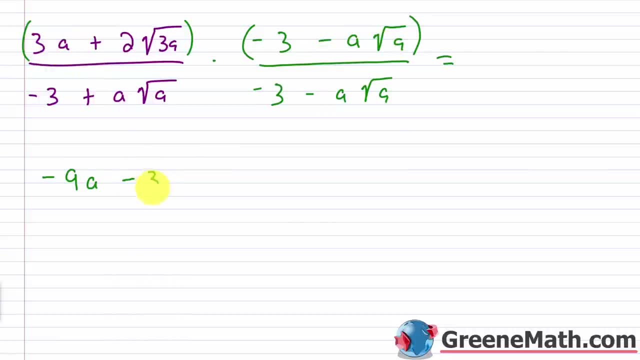 of a. So that's going to be negative. 3a times a is 3a squared and then times square root of a For the inner, I've got 2 times square root of 3a times negative 3.. So that's negative. 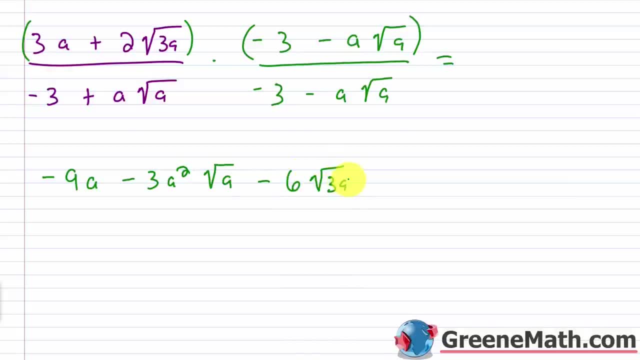 6 times square root of 3a. And then And then for the last, I'm going to have 2 times negative a or negative 2a times the square root of 3a. times the square root of a. 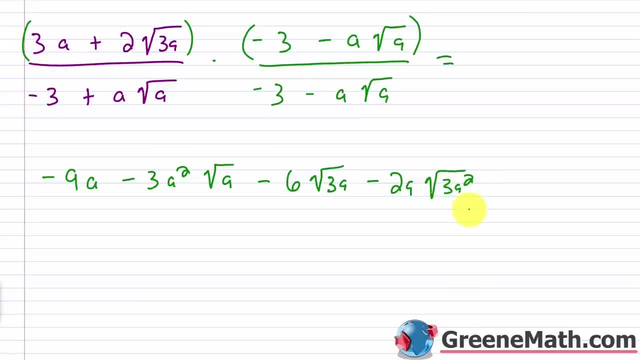 So that would be the square root of 3a squared. So I know the square root of a squared is a, So I can pull that out and make this a squared times the square root of 3.. Now is there anything I can do to simplify here? 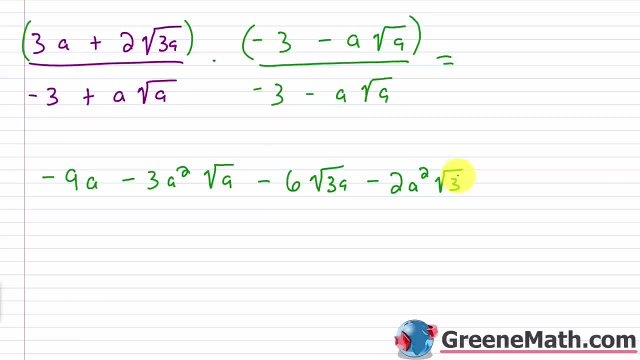 No, there's not. There's nothing else I can do. I know it's long, but there's nothing I can do to simplify. So then, this is over. Now I'm going to use my special products formula here, and that tells me to take the first. 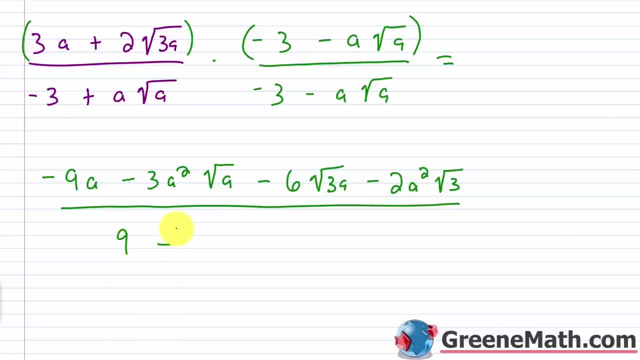 guy and square it. Negative, 3 squared is 9.. And then minus the second guy squared. So then that would be a squared times square root of a. times square root of a would be a. So really a squared times a or a cubed. 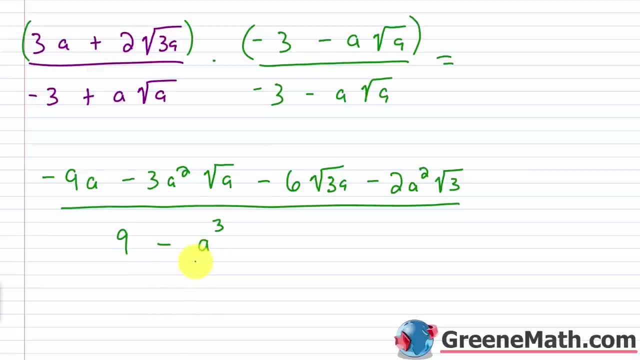 So my denominator becomes 9 minus a cubed. Nothing I can do with that. So I have negative 9a minus 3a, squared times square root of a Minus 6 times square root of 3a minus 2a, squared times square root of 3 over 9 minus a cubed. 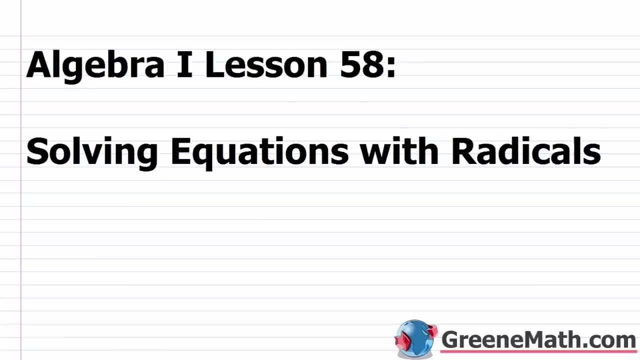 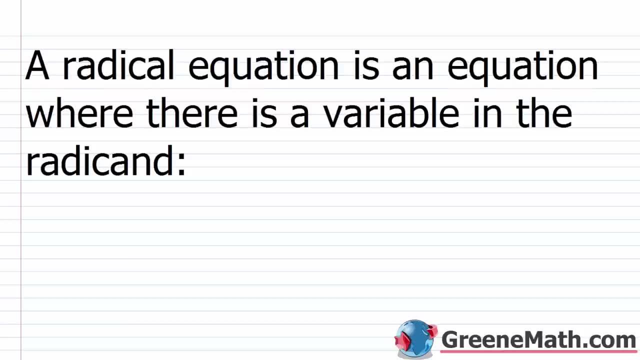 as my simplified answer. Hello and welcome to Algebra 1, lesson 58.. In this video we're going to learn about solving equations with radicals. So a radical equation is an equation where there is a variable in the radicand. So let me repeat that. 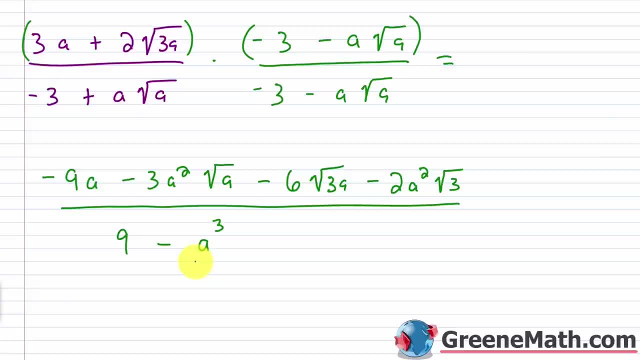 second guy squared. Nothing I can do with that. So I have negative 9a minus 3a squared times square root of a minus 6 times square root of 3a minus 2a squared times square root of 3 over 9 minus a 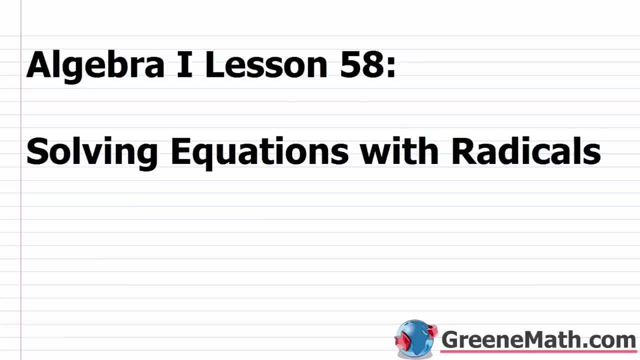 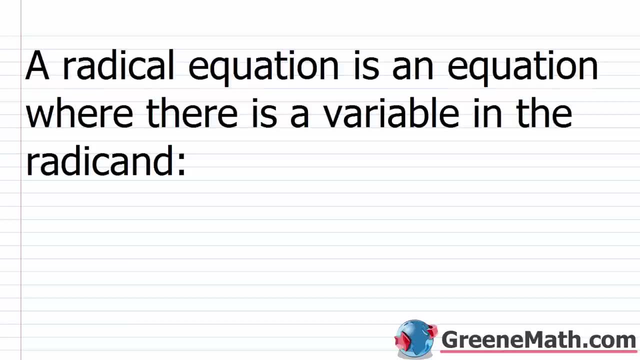 cubed as my simplified answer. Hello, and welcome to Algebra 1 Lesson 58. In this video, we're going to learn about solving equations with radicals. So a radical equation is an equation where there is a variable in the radicand. 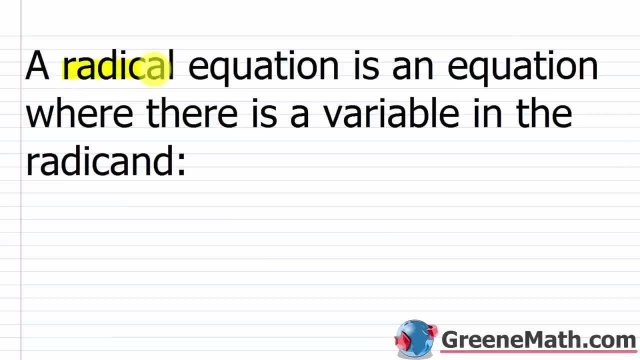 So let me repeat that. A radical equation is an equation where there is a variable in the radicand. So I know most of you know this. But in case you don't, because you might be saying, what's a radicand? Again, if we had something like a square root, or a cube root, or fourth root, or whatever it is, let's just go with a square root because that's the most common. The radicand is the number or the variable. So if we had something like a square root, or a cube root, or the you could say expression that's underneath that symbol. So something like square root of 3x. This would be your radicand. So again, a radical equation, one more time, is an equation where there is a variable in the radicand. So as an example, we see something like the square root of x plus 2 equals 5. 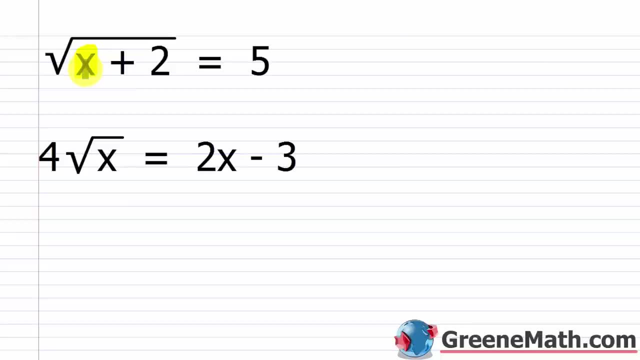 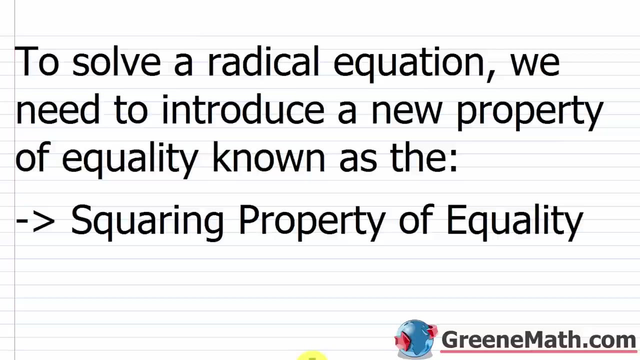 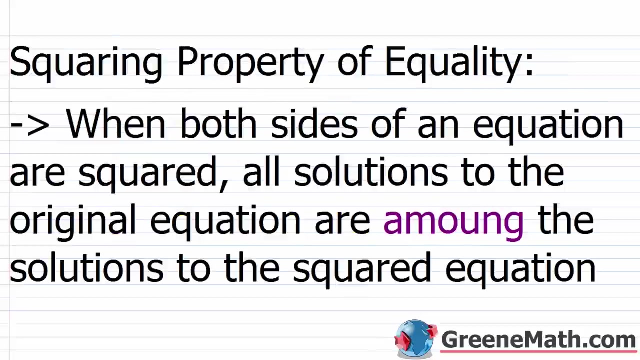 The radicand, you have that variable x. As another example, we have 4 times the square root of x is equal to 2x minus 3. Here, the radicand just consists of x. But that's a variable. And so this is a radical equation. All right. So in order to solve a radical equation, we need to introduce a new property of equality known as the squaring property of equality. We've also learned the addition property of equality and the multiplication property of equality. So this is just another tool in our chest, you know, to solve equations moving forward. So the squaring property of equality. There's one kind of little hiccup to this thing. When both sides of an equation are squared, all solutions to the original equation are among, okay, among the solutions to the squared equation. 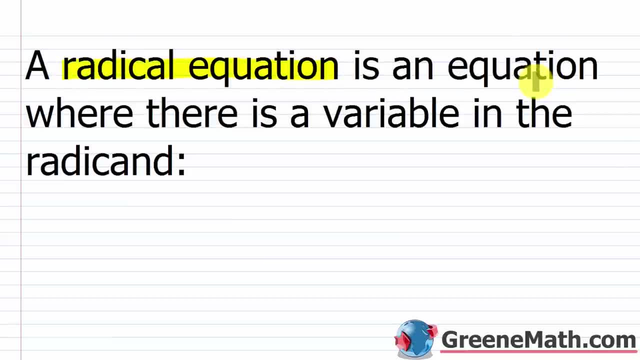 A radical equation is an equation where there is a variable in the radicand. So I know most of you know this, but in case you don't, because you might be saying what's a radicand again if we had something like a square root or cube root or fourth root, 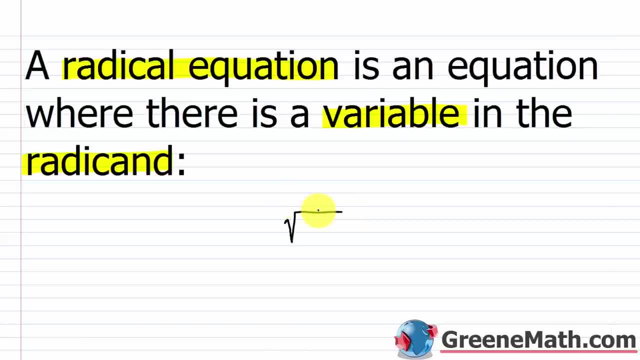 or whatever it is. let's just go with a square root because that's the most common. the radicand is the number or the variable or the- you could say- expression that's underneath that symbol. So something like square root of 3x. 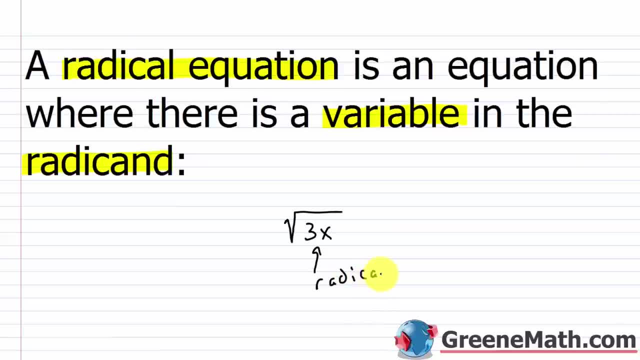 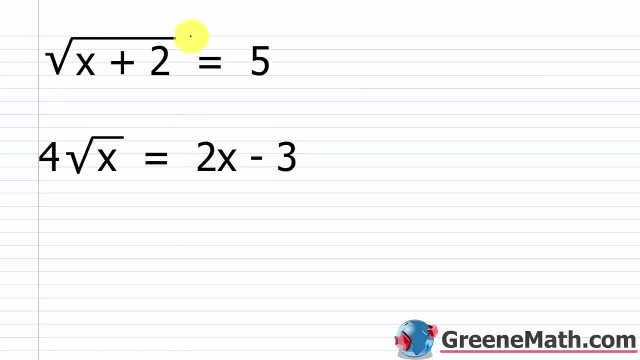 This would be your radicand. So again, a radical equation. one more time is an equation where there is a variable in the radicand. So as an example, we see something like the square root of x plus 2 equals 5.. 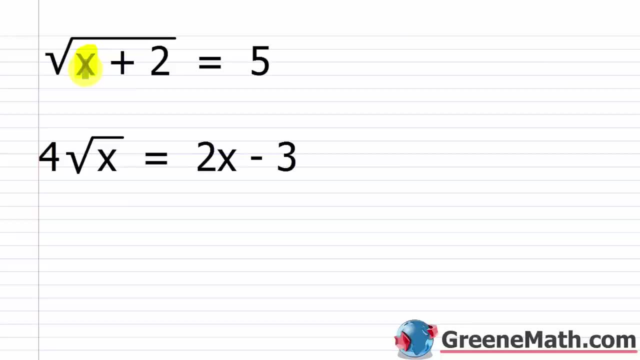 In your radicand you have that variable x. As another example, We have 4 times the square root of x. The square root of x is equal to 2x minus 3.. Here the radicand just consists of x, but that's a variable, and so this is a radical. 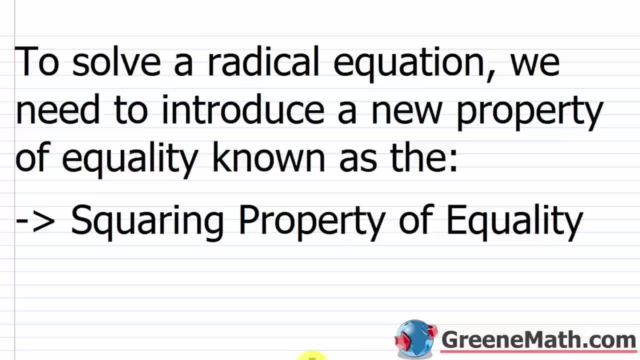 equation, All right. so in order to solve a radical equation, we need to introduce a new property of equality, known as the squaring property of equality. We've also learned the addition property of equality and the multiplication property of equality, So this is just another tool in our chest. 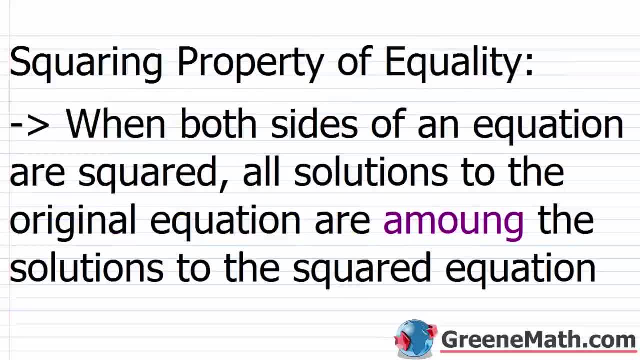 You know, to solve equations moving forward. So the squaring property of equality. There's one kind of little hiccup to this thing. When both sides of an equation are squared, all solutions to the original equation are among, okay, among the solutions to the squared equation. 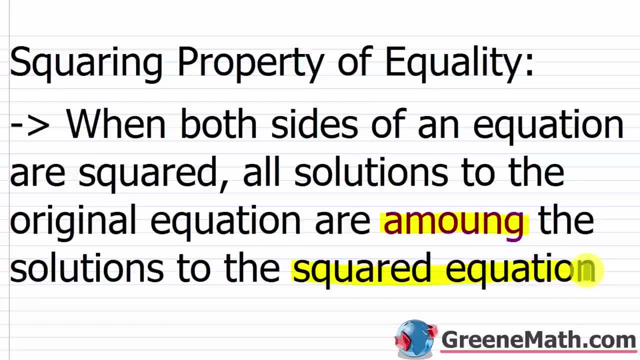 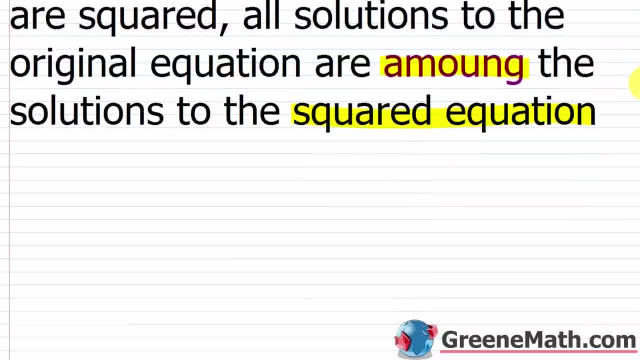 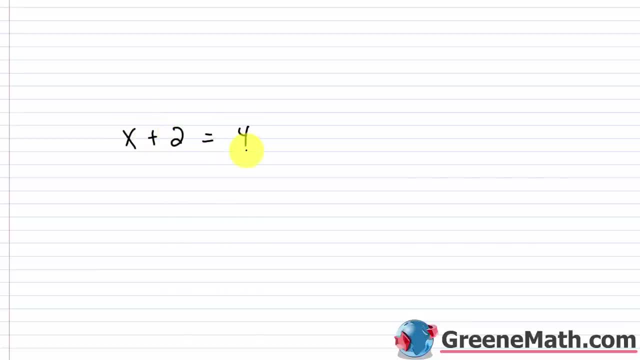 Now that seems like it's not a big deal, but it really kind of is. If I use something like the addition property of equality. As we recall, that looks like this. Let me kind of scroll down: We have x plus 2 equals 4 as an example. 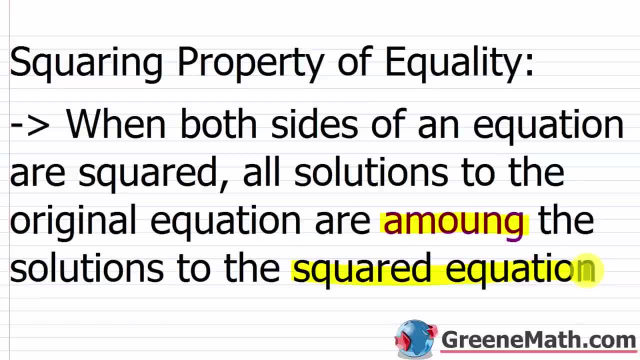 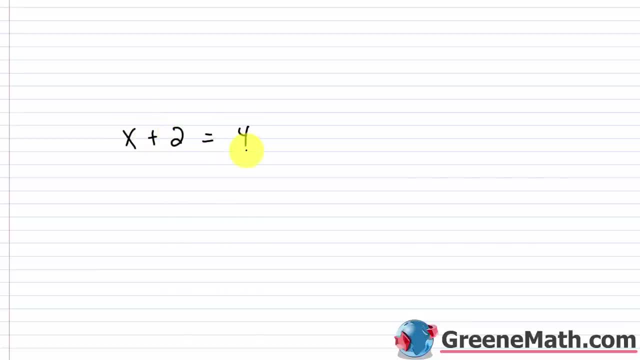 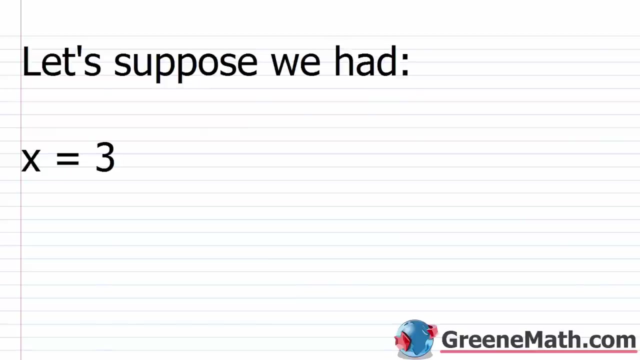 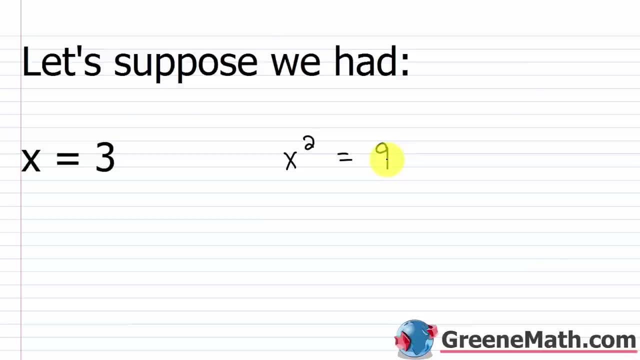 equation so we can kind of, you know, mentally figure out what this is. What squared would give me 9? Well, I know 3 does, right? 3 squared would be 9. 3 times 3 is 9. But I also know that negative 3 squared would give me 9 as well. So the solution for this equation, for this equation, would be x equals 3 or x equals negative 3. So there's two solutions there. But in the original equation, if I took this negative 3 and I plugged it in for x here, we'd have a big problem. We'd have negative 3 is equal to 3. That's false. That does not work. So let me kind of line this out and say wrong. Okay, that's wrong. So you can see that when we squared that equation, we came up with an equation that had solutions that did not work in the original one. So that's 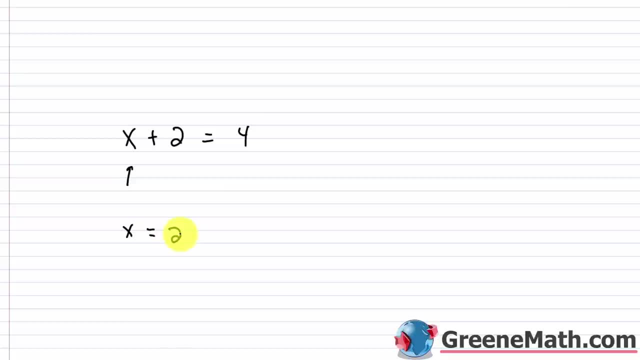 I know the solution to this equation is x equals 2.. If I added 3 to both sides of the equation- so let's say I add 3 over here- That would make this 5.. I add three over here, That would make the 7.. 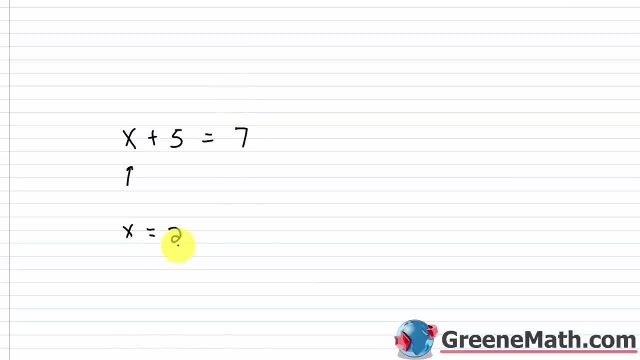 The solution is still: x equals 2. Still works out if I have the multiplication property of equality. So something like, let's say, 3x equals 12. I know this is x equals 4.. If I multiply both sides by negative 2, this would be negative 6x and this would be negative 24.. 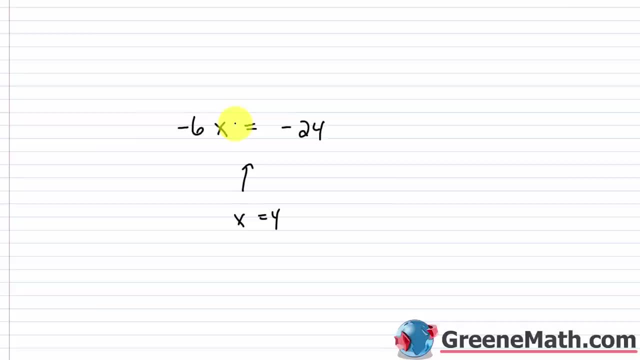 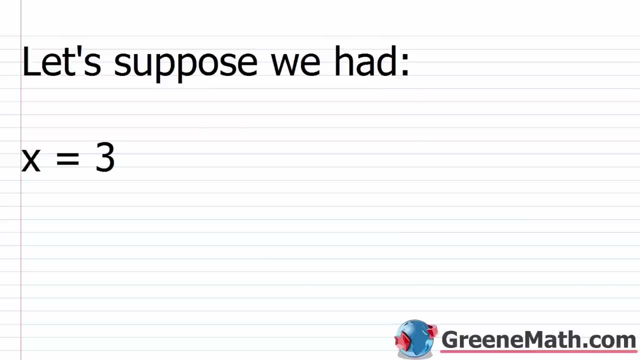 x equals 4 is still a solution. Log in a 4. there you get a true statement With the squaring property of equality. this is not always going to be true, So let's suppose we had x equals 3.. Very, very simple. 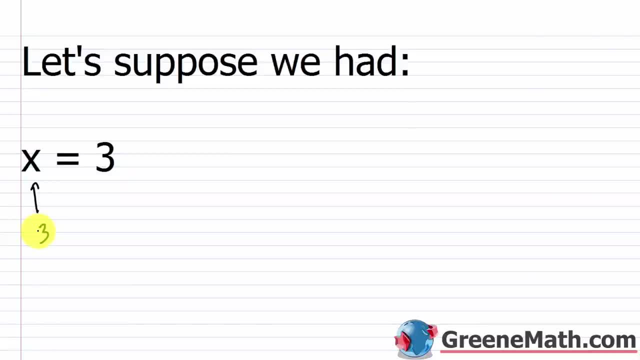 I know that if I replace x with 3, I get a true statement. But let's say I square both sides of this, So x becomes squared and 3 becomes squared. So now I have x squared equals 9.. Now we haven't covered how to solve an equation like this yet, but let's just think about it. 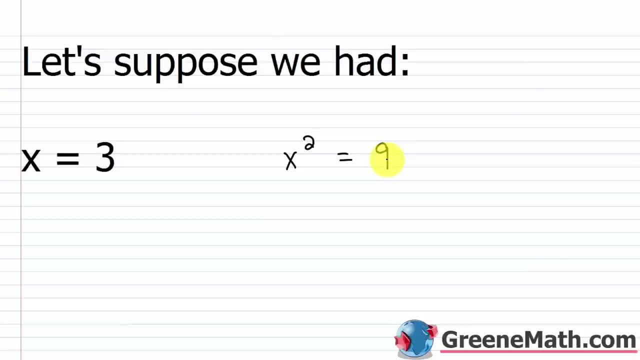 It's a very, very simple equation, so we can kind of mentally figure out what this is. What squared would give me 9?? Well, I know, 3 does right. 3 squared would be 9.. 3 times 3 is 9.. 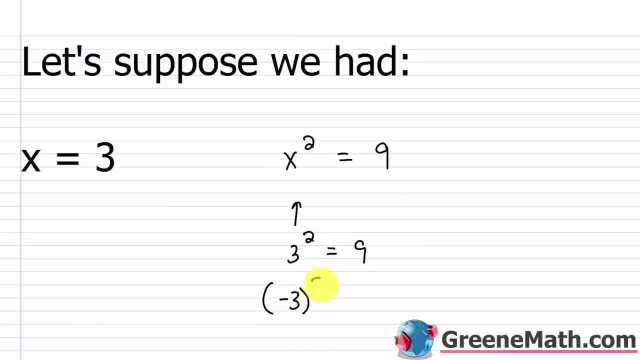 But I also know that negative 3 squared would give me 9 as well. So the solution for this equation for this equation would be x equals 3 or x equals negative 3.. So there's two solutions there. But in the original equation, if I took this negative 3,, 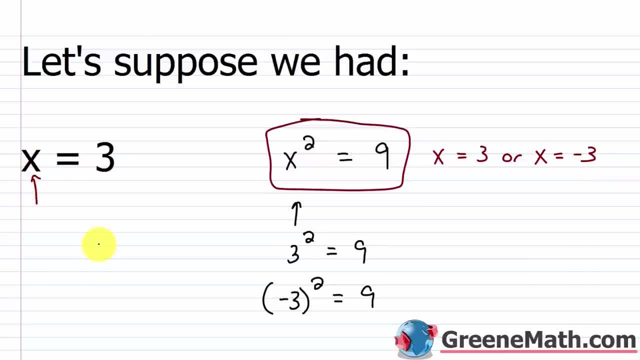 and I plugged it in for x. here we'd have a big problem. We'd have negative. 3 is equal to 3.. That's false. That does not work. So let me kind of line this out and say: wrong, Okay, that's wrong. 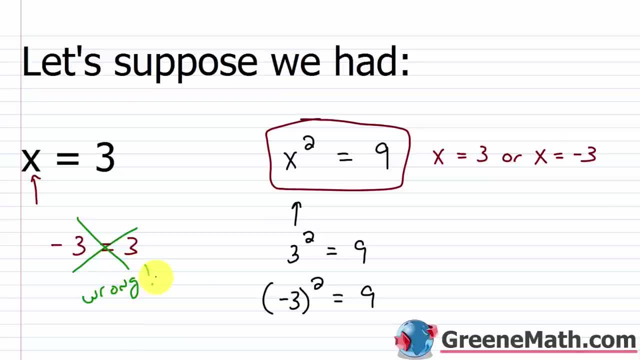 So you can see that when we squared that equation, we came up with an equation that had solutions that did not work in the original one. So that's why it's very, very important that when you use the squaring property of equality, you have to check each and every solution that you generate. 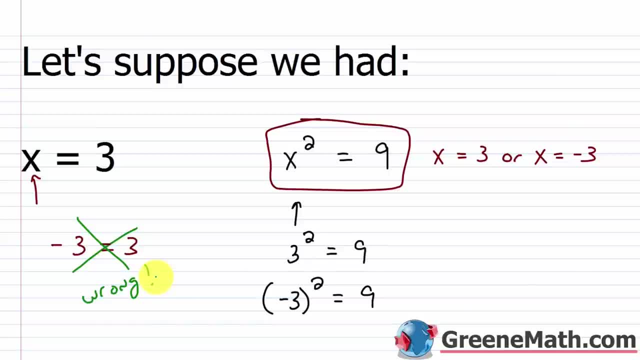 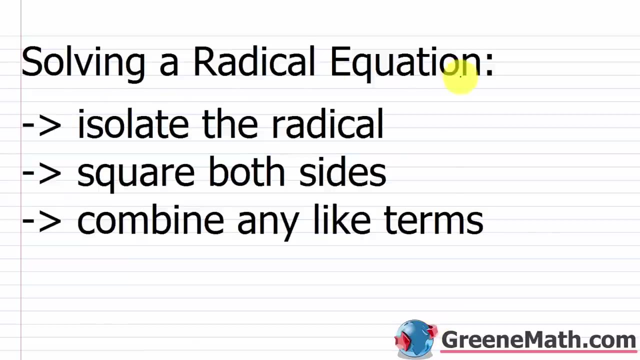 why it's very, very important that when you use the squaring property of equality, you have to check each and every solution that you generate in order to make sure it works in the original equation. All right, so now let's just take a look at the procedure to solve a radical equation. So I have solving a radical equation. We want to isolate the radical. So that's the first thing you're going to do. 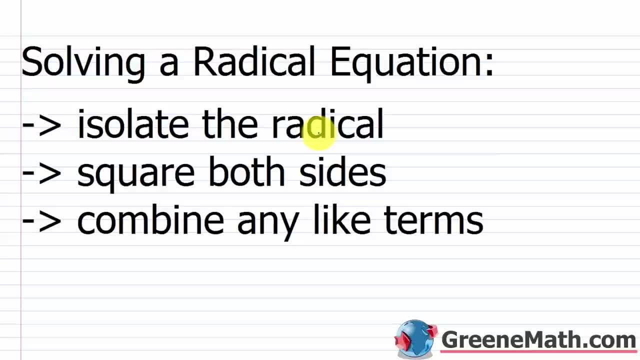 Now, in the most complicated situations, you're going to have more than one radical involved. And in that case, you just want to isolate one radical at a time. Now, the next step is going to depend on what type of root you're looking at. Do you have a square root? Do you have a cube root? Do you have a fourth root? In algebra one, we're just going to deal with square roots. 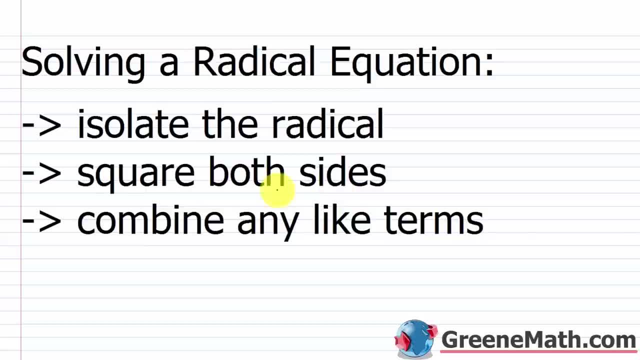 So I just put square both sides. So we would square both sides in the case of a square root. Then we would combine any like terms. Now, at this point, we're going to have a square root. So we're going to have a square root. 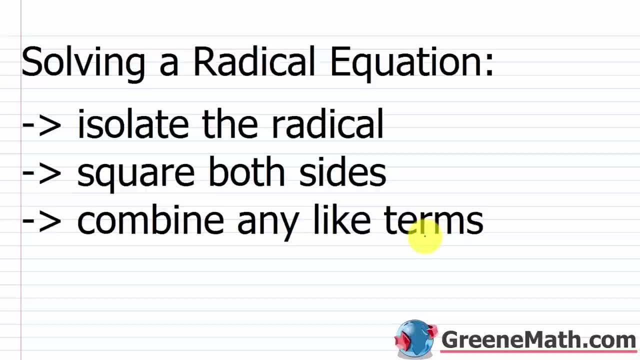 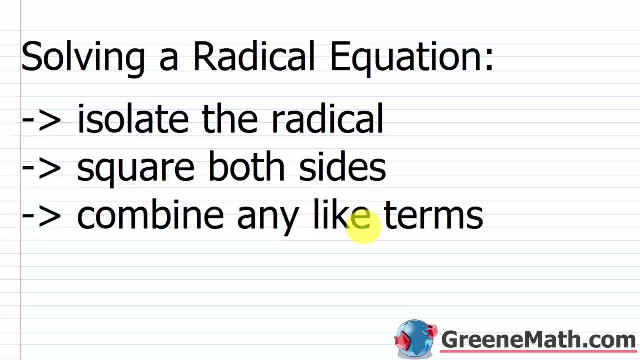 At this point, if you had any radicals that remained, you're going to go back up to this first step, and you're going to come back down. You're going to keep doing that until you're radical free. Then lastly, you're going to solve the equation and check all potential solutions 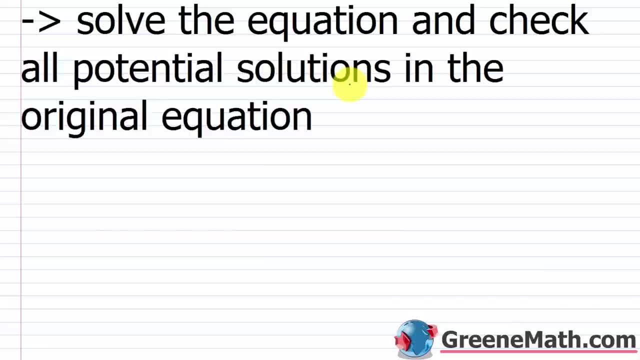 in the original equation. And again, this is very, very important. Check all potential solutions in the original equation. It's not going to happen to you every time, but at least sometimes, the solutions you're going to get from that transformed equation is going to give you problems or not work in that original one. And so it's not going to be a solution that you can use as an answer for your problem. All right, let's start out with something very, very easy. 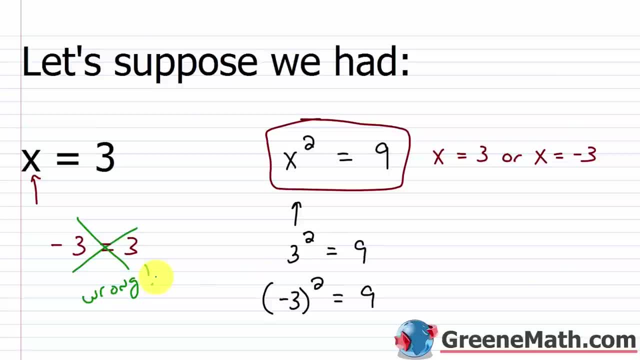 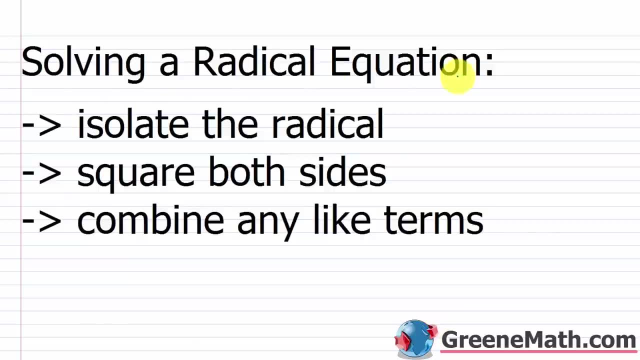 in order to make sure it works in the original equation. All right, so now let's just take a look at the procedure to solve a radical equation. So I have solving a radical equation. We want to isolate the radical, So that's the first thing you're going to do. 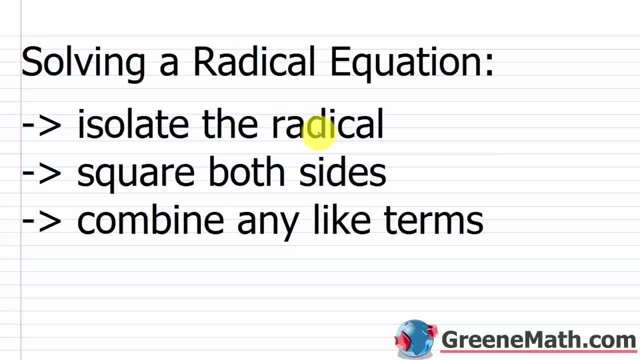 Now, in the most complicated situations, you're going to have more than one radical involved, And in that case, you just want to isolate one radical at a time. Now the next step is going to depend on what type of root you're looking at. 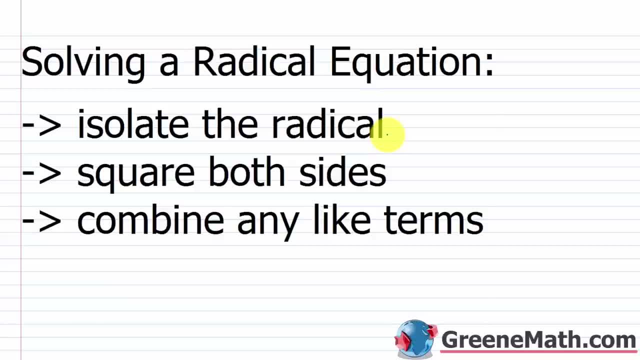 Do you have a square root? Do you have a cube root? Do you have a fourth root In algebra one? we're just going to deal with square roots, So I just put square both sides. So we would square both sides in the case of a square root. 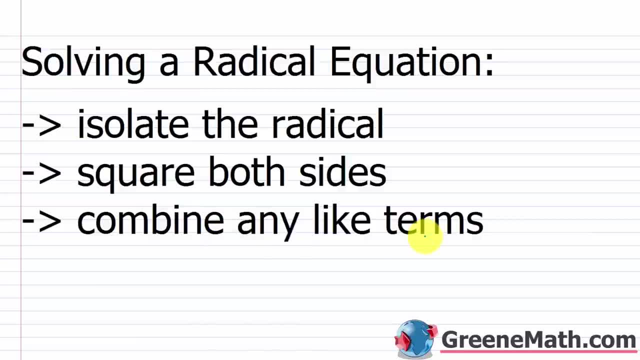 Then we would combine any like terms. Now, at this point, if you had any radicals that remained, you're going to go back up to this first step and you're going to come back down. You're going to keep doing that until you're radical free. 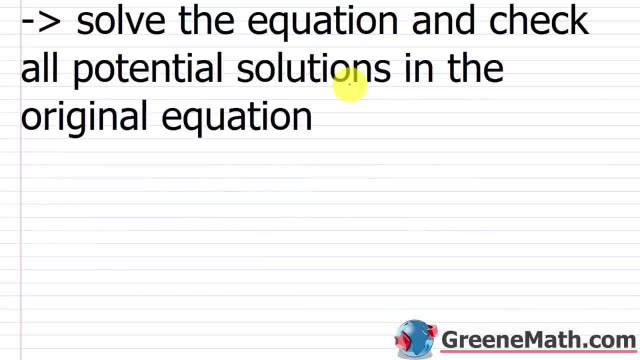 Then, lastly, you're going to solve the equation and check all potential solutions in the original equation. Okay, And again, this is very, very important: Check all potential solutions in the original equation. It's not going to happen to you every time. 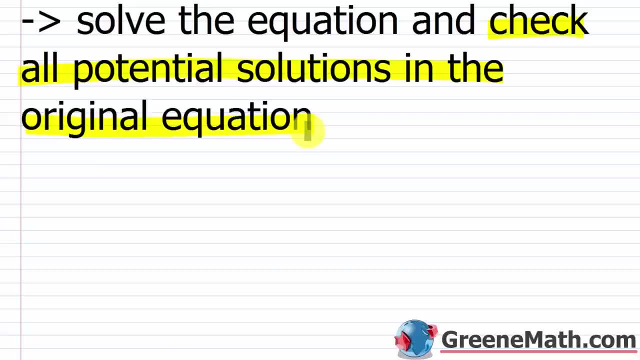 but at least sometimes the solutions you're going to get from that transformed equation is going to give you problems or not work in that original one, And so it's not going to be a solution that you can use. It's going to be a solution that you can use to solve your problem. 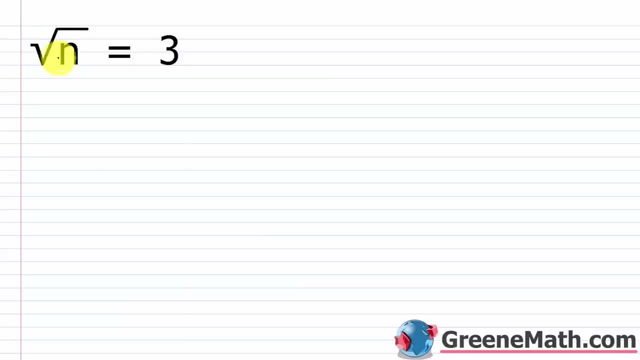 All right, Let's start out with something very, very easy. So we have: the square root of n is equal to three, So the radical is already isolated here. Okay, So I don't need to do that step And I would just start out by just squaring both sides. 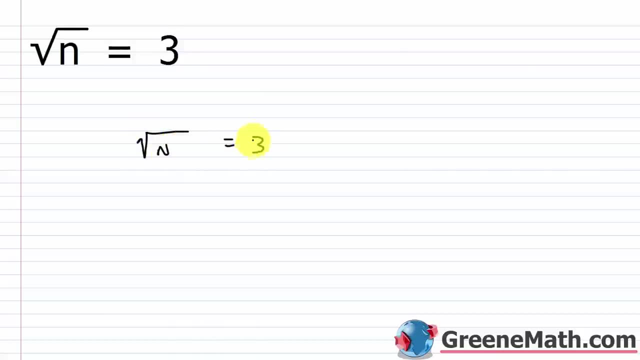 So if I have the square root of n is equal to three and I square this side and I square this side, what's going to happen is we know that this cancels with this, because we just have n and three squared is nine. 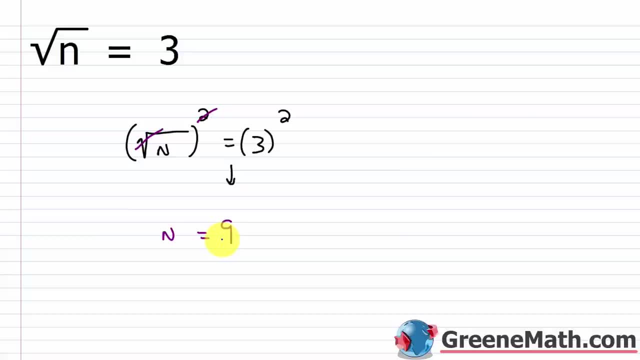 So n equals nine. I get one solution there, So plug this back in for n. If I plugged in a nine there, what would I have I would have? the principal square root of nine is equal to three, And that is true, right. 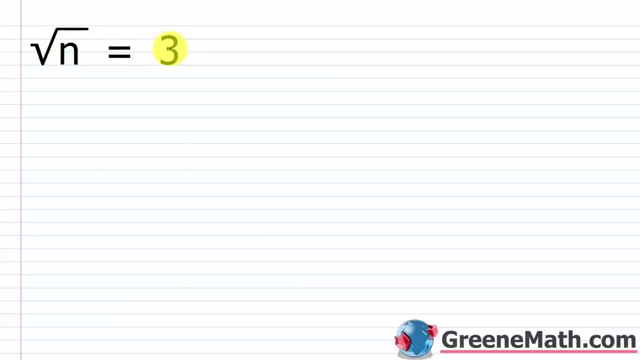 So we have the square root of n is equal to three. So the radical is already isolated here. Okay, so I don't need to do that step. And I would just start out by just squaring both sides. So if I have the square root of n is equal to three, and I square this side, and I square this side, what's going to happen is we know that this cancels with this, and I just have n, and three squared is nine. So n equals nine. I get one solution there. So plug this back in for n. If I plugged in a nine there, what would I have? I would have the principal square root of nine is equal to three. And that is true, right? 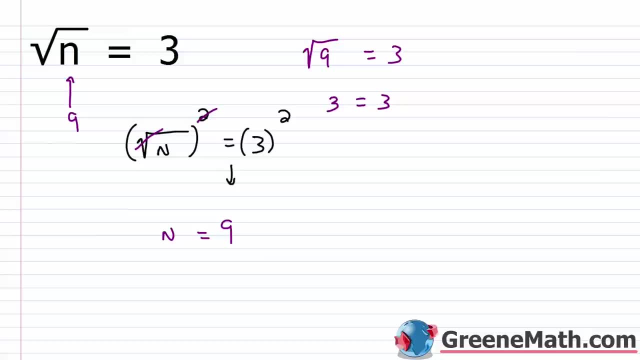 Square root of nine is three. You get three equals three. So this checks out as a solution. 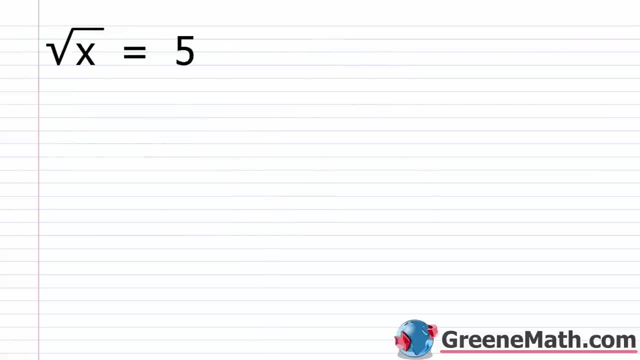 Let's take a look at another easy one. So we have that the square root of x is equal to five. 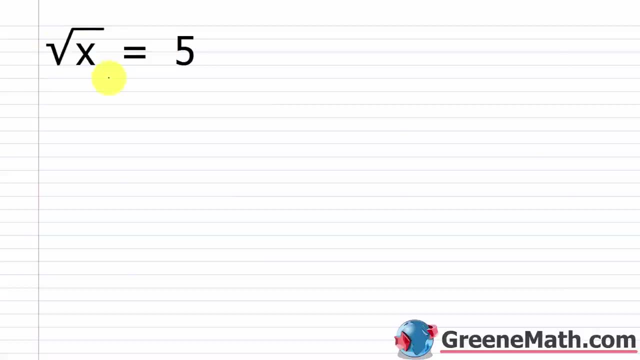 Again, the radical is already isolated for me. I don't need to do that. And so all I need to do is just square both sides of the equation. 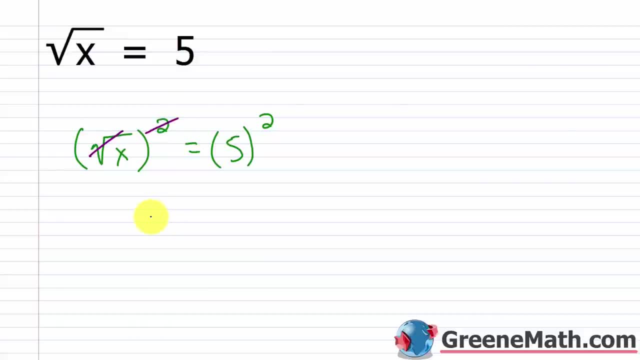 And so what's that going to give me? Well, this is going to cancel with this, and I'll just have x. Five squared is 25. 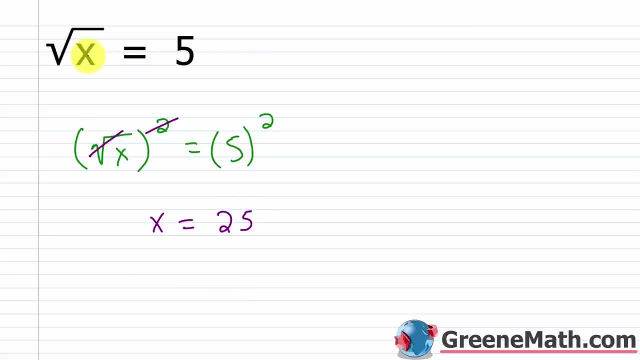 Solution only. And so again, if I plug in a 25 for x there, the square root of 25, we all know that's five. So this is a valid solution. Let's look at one that's a little 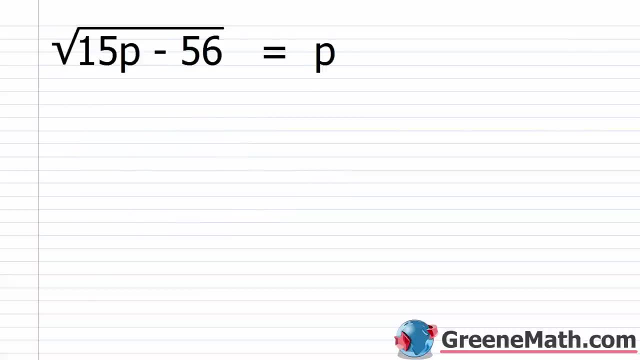 bit more challenging. So we have the square root of 15p minus 56 is equal to p. So the radical, again, is isolated for me. So what I'm going to do is I'm going to, again, square both sides. This equals p. So I'm going to... 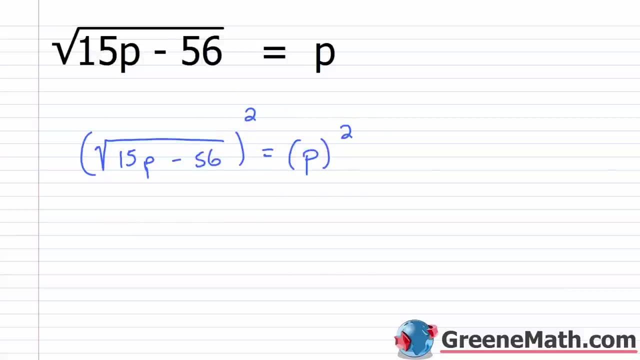 I'm going to square this side, and I'm going to square this side. Okay. So if I square this, this cancels with this, and I'm left with the radical. So I'm left with 15p minus 56, and this equals p squared. So what we have now is a quadratic equation. And we've worked with 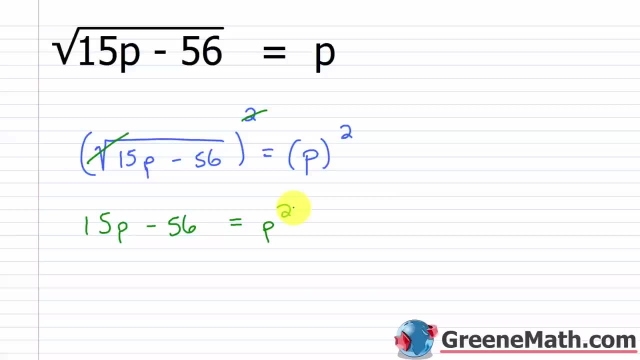 these in a previous lesson, and I taught you how to solve them when they're factorable. We have not gotten to the point to where you have a quadratic equation, it's not factorable, you know how to solve it. So we have a quadratic equation, and we have a quadratic equation, you know how to solve it. We're going to get to that when we start talking about completing the 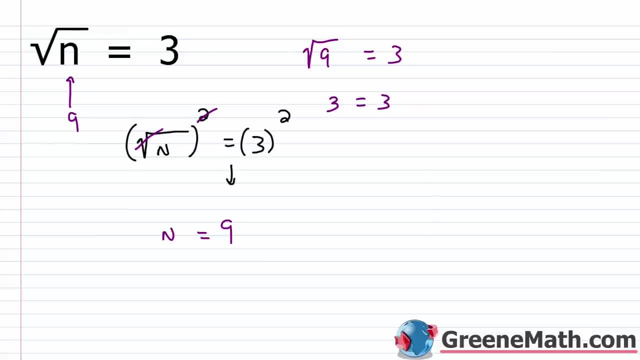 Square root of nine is three. You get three equals three, So this checks out as a solution. Let's take a look at another easy one. So we have that the square root of x is equal to five. Again, the radical is already isolated. for me, 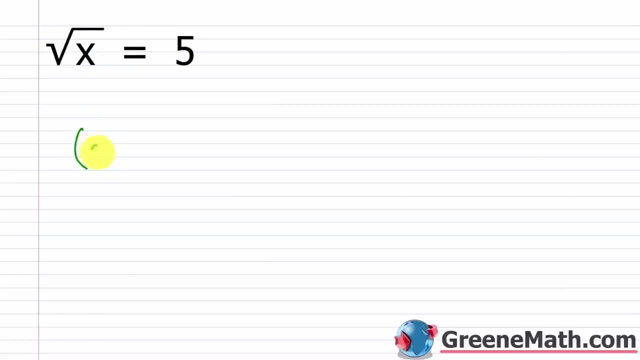 I don't need to do that, And so all I need to do is just square both sides of the equation. And so what's that going to give me? Well, this is going to cancel with this, and I'll just have x five squared is 25.. 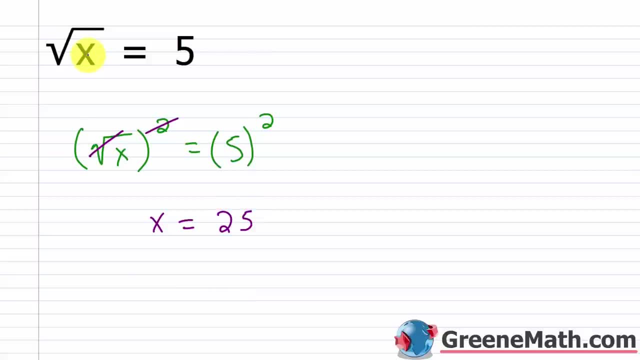 I get one solution only, And so again, if I plug in a 25 for x, there, the square root of 25, we all know that's five. So this is a valid solution. Let's look at one that's a little bit more challenging. 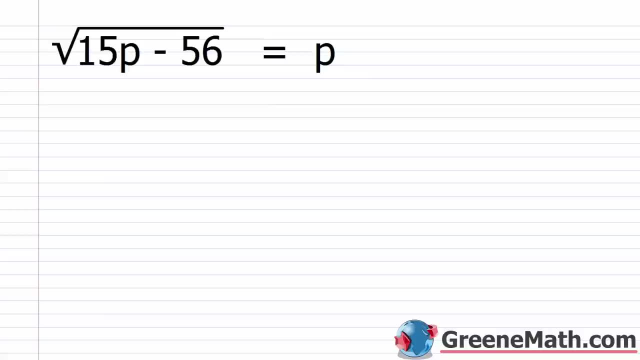 So we have the square root of 15p minus 56 is equal to p, So the radical again is isolated for me. So what I'm going to do is I'm going to again square both sides. This equals p. So I'm going to square this side and I'm going to square this side. 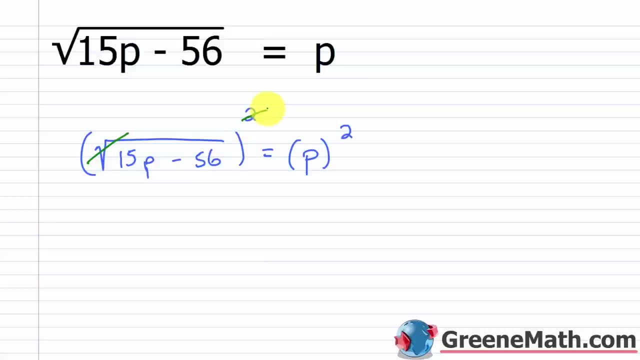 Okay. So if I square this, this cancels with this and I'm left with the radicand. So I'm left with 15p minus 56.. And this equals p squared. So what we have now is a quadratic equation. 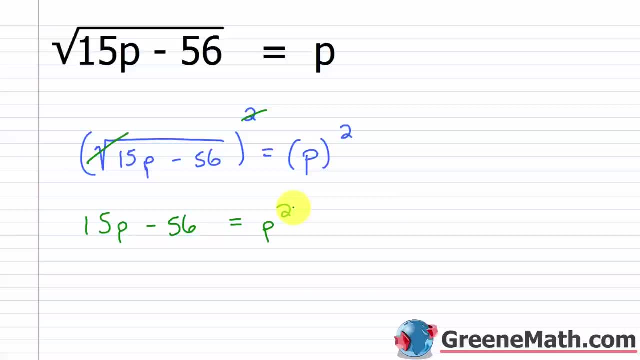 And we've worked with these in a previous lesson And I taught you how to solve them when they're factorable. We have not gotten to the point to where you have a quadratic equation. It's not factorable. You know how to solve it. 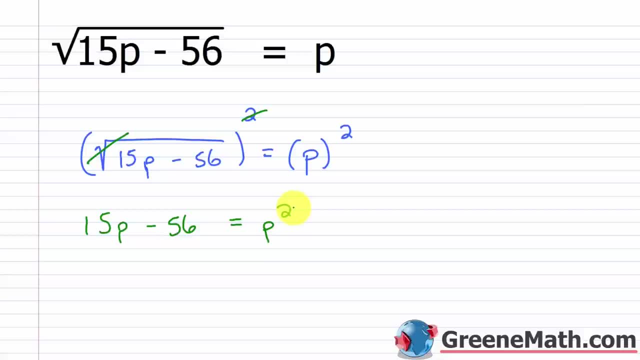 We're going to get to that when we start talking about completing the square and then the quadratic formula. That's going to be the very last lessons of Algebra 1.. So for this lesson, I gave you stuff that you could factor. All right. 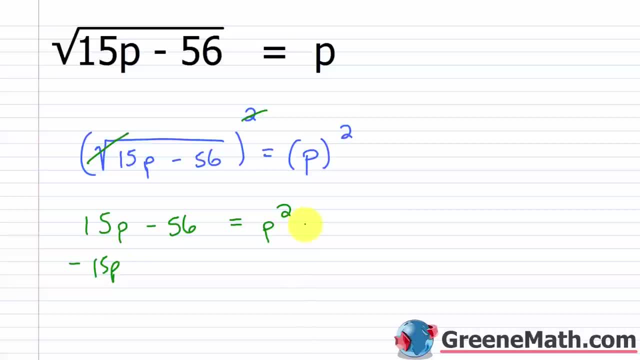 So for this I'm just going to subtract 15p away from both sides. I'm going to add 56 to both sides And that's going to make this side equal to 0. So what I'm going to have. let me scroll down here a little bit. 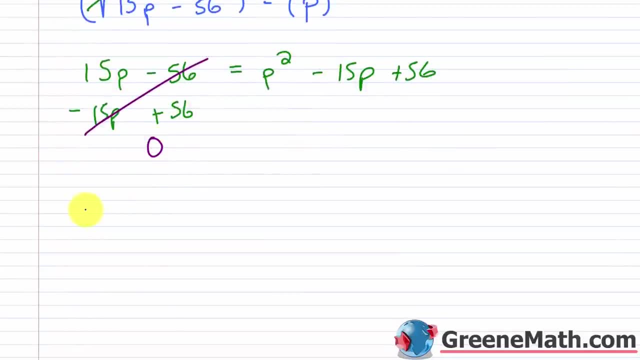 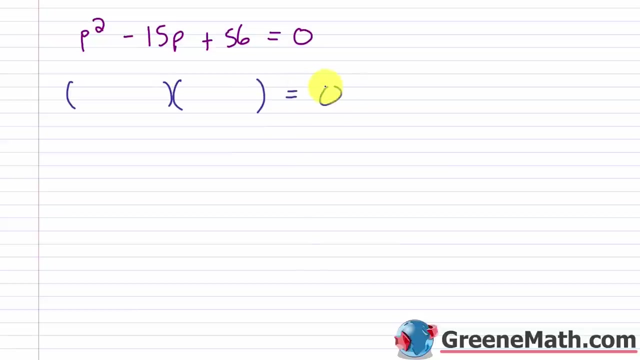 And I like 0 to be on the right side, So let me move everything over. So I would have p squared minus 15p plus 56 is equal to 0. And I'm going to factor My left side. Okay, so I need two integers whose sum is going to be negative 15 and whose 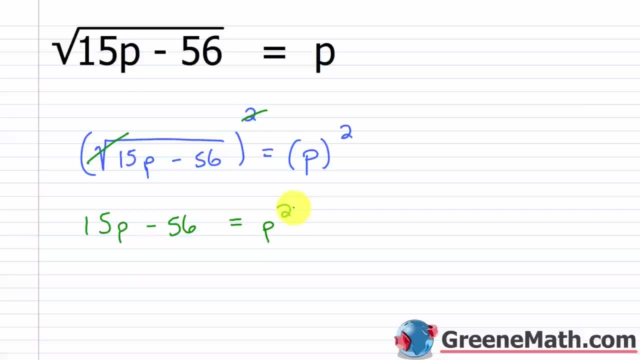 square and then the quadratic formula. That's going to be the very last lessons of Algebra 1. So for this lesson, I gave you stuff that you could factor. All right. So for this, 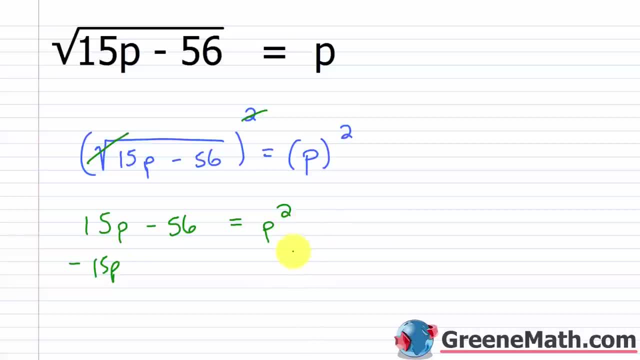 I'm just going to subtract 15p away from both sides. I'm going to add 56 to both sides. 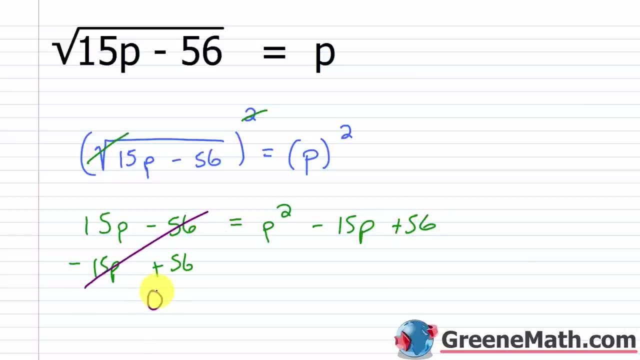 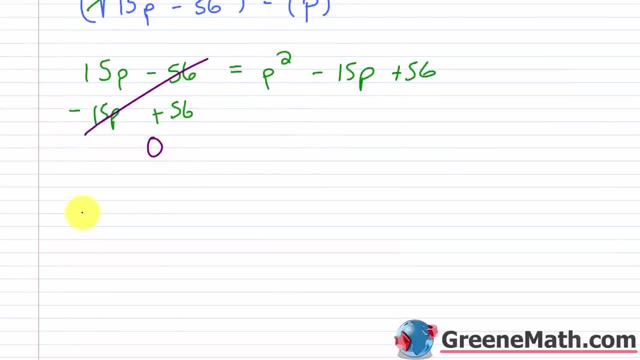 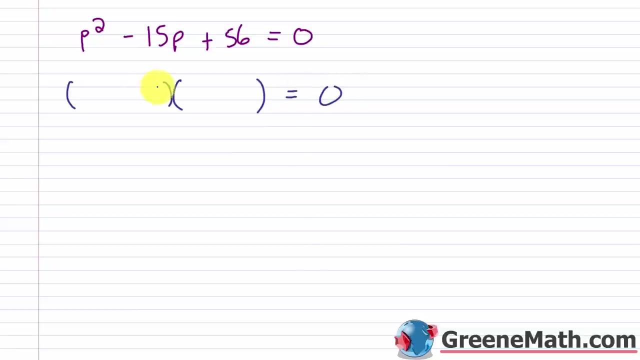 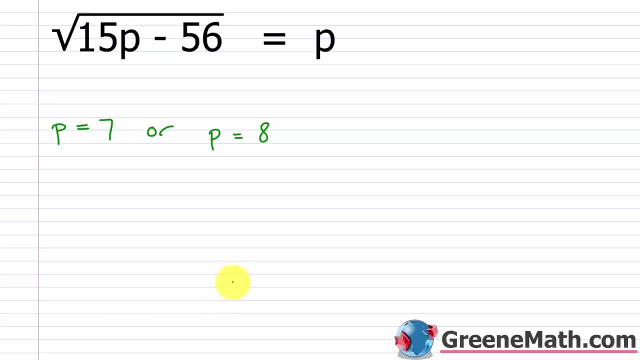 And that's going to make this side equal to zero. So what I'm going to have, let me scroll down here a little bit. And I like to do this. I'm going to subtract 15p away from both sides. And I'm going to like zero to be on the right side. So let me move everything over. So I would have p squared minus 15p plus 56 is equal to zero. And I'm going to factor my left side. Okay, so I need two integers, whose sum is going to be negative 15, and whose product is 56, going to be negative seven and negative eight. So minus seven minus eight. So we know how to solve this, we take each factor, okay, that had a variable involved, we'd set it equal to zero. It's called the zero product property. Okay, so we'd have p minus seven equals zero. And then also we can put or p minus eight equals zero, add seven to both sides here, add eight to both sides here, and we get p is equal to seven or p is equal to eight. Now, we're not done because we need to check this in the original equation. So if I plug in, a seven for p there, I would have the square root of 15 times seven, which is 105 minus 56. 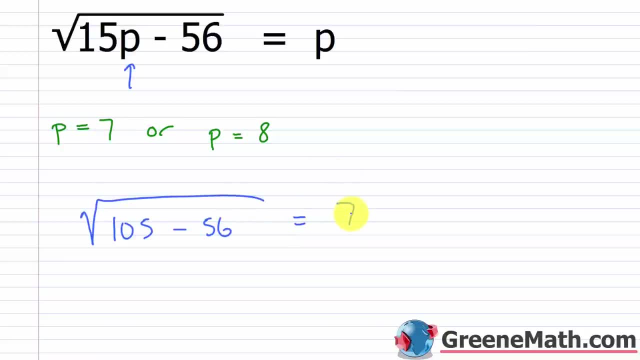 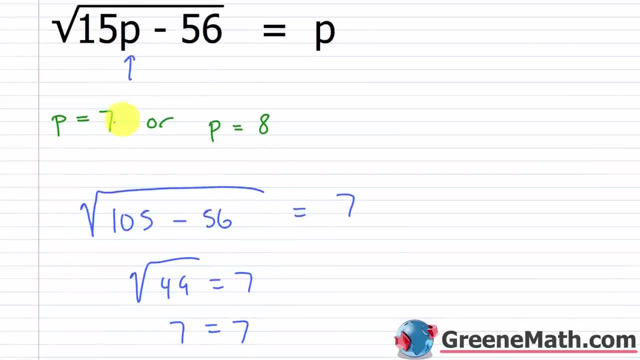 And this should be equal to seven. So 105 minus 56 is 49. We know that the square root of 49 is seven, right, this would give me seven equals seven. So that's a valid solution. 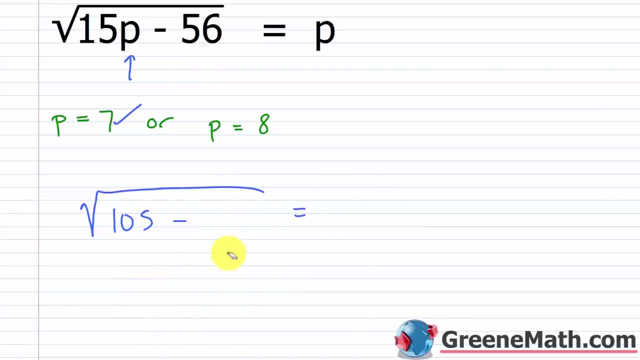 For the next one, we have eight. Okay, so let's try that out. This stays the same. 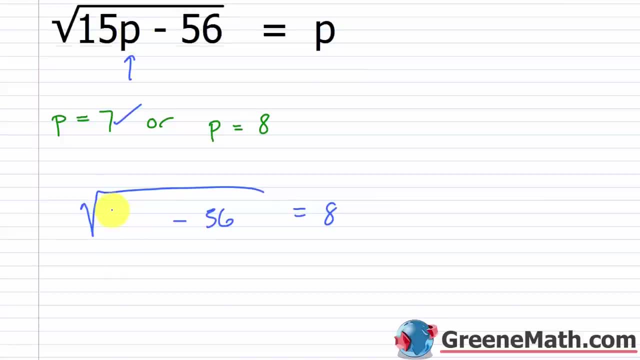 And 15, times eight now will give me 120. So if I do the square root of 120 minus 56, that's the square root of 64. 120 minus 56 is 64. So this would be the square root of 64 is equal to eight. And we 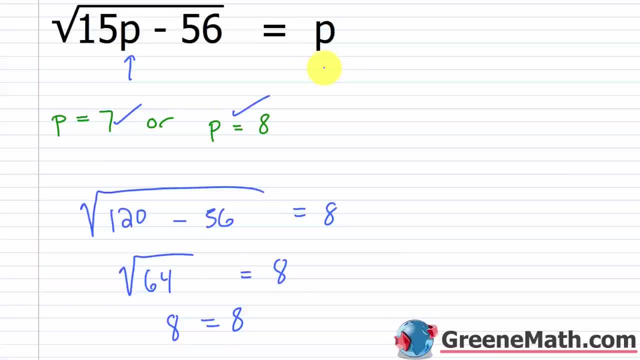 know that's true, right? This would be eight equals eight. So this is a valid solution as well. So 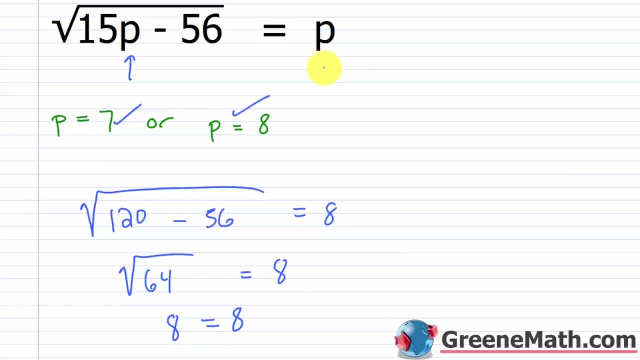 here p equals seven or p equals eight. Let's take a look at another one. So we have the square root 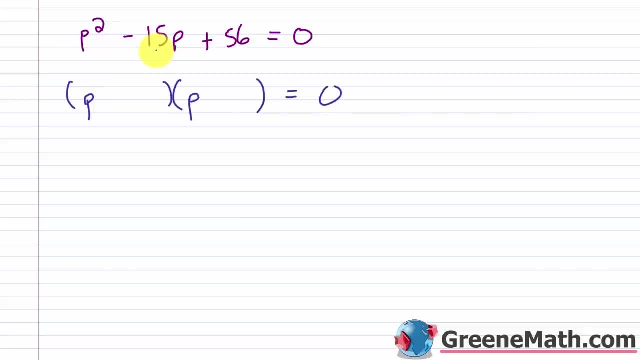 product is 56.. It's going to be negative 7 and negative 8.. So minus 7, minus 8.. So we know how to solve this. We take each factor. Okay that had a variable involved, We'd set it equal to 0.. 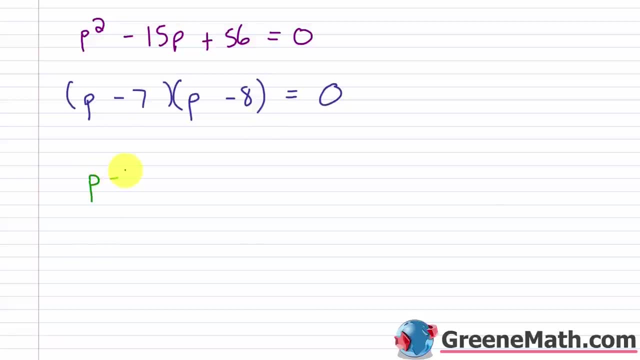 It's called the zero product property. Okay, so we'd have: p minus 7 equals 0.. And then also we can put: or p minus 8 equals 0.. Add 7 to both sides here. add 8 to both sides here. 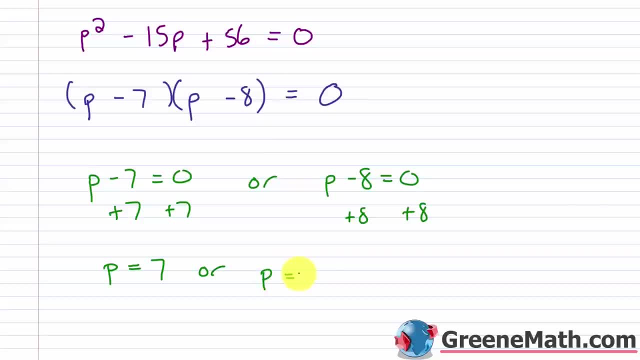 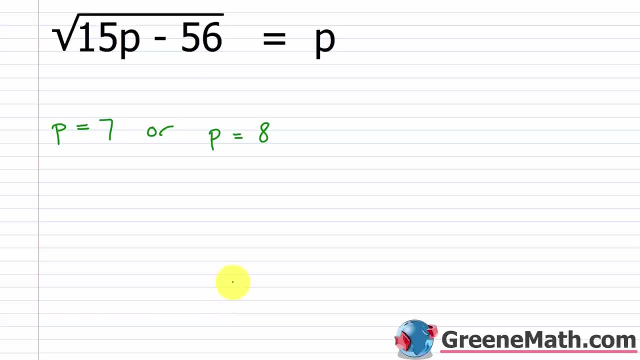 And we get p is equal to 7 or p is equal to 8.. Now we're not done because we need to check this in the original equation. So if I plug in a 7 for p there, I would have the square root of 15 times 7, which is 105 minus 56.. 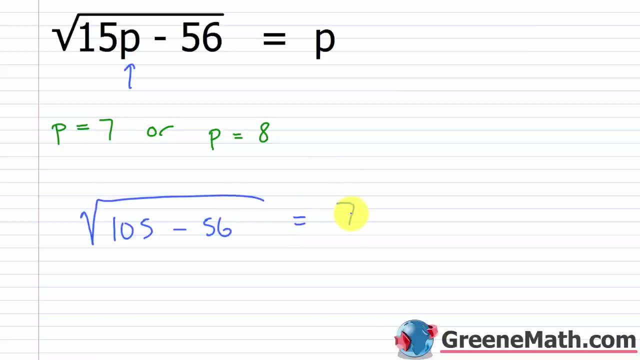 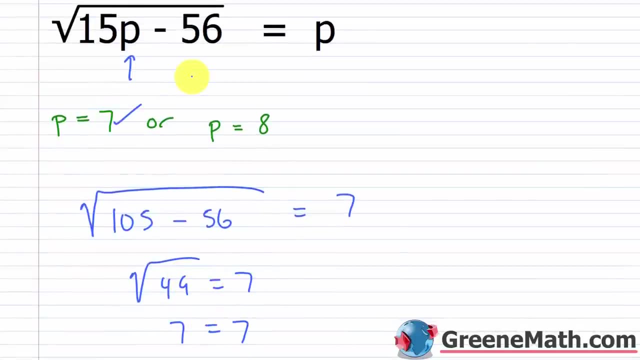 And this should be equal to 7.. So 105 minus 56 is 49.. We know that the square root of 49 is 7, right, This would give me 7 equals 7.. So that's a valid solution. 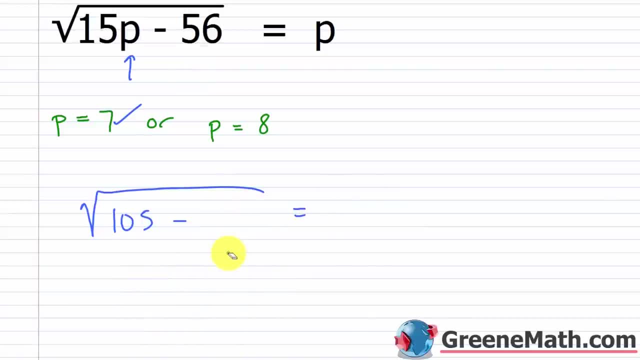 For the next one we have 8.. Okay, so let's try that out. This stays the same, And 15 times 8 now would give me 120.. So if I do the square root of 120 minus 56, that's the square root of 64.. 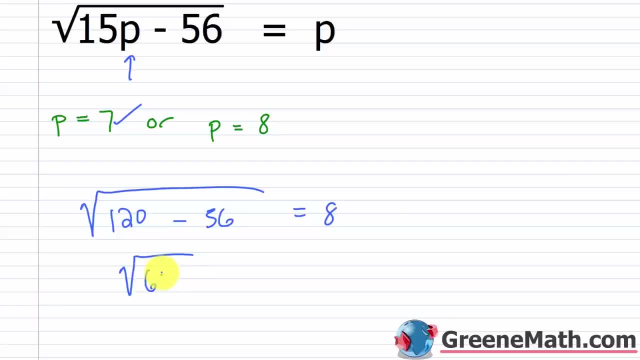 120 minus 56 is 64.. So this would be: the square root of 64 is equal to 8.. And we know that's true, right. This would be 8 equals 8.. So this is a valid solution as well. 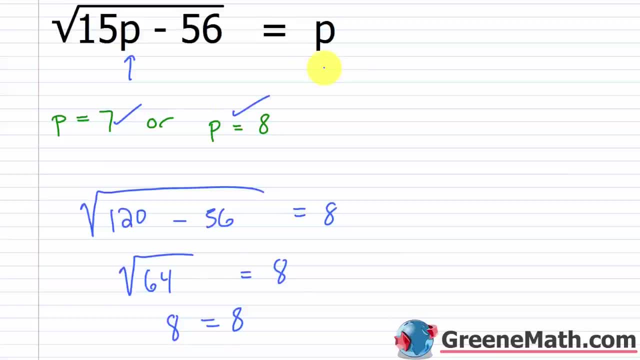 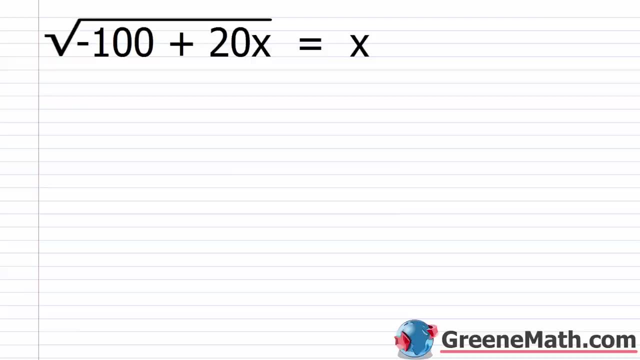 So here p equals 7 or p equals 8.. Let's take a look at another one. So we have the square root of negative. 100 plus 20x is equal to x. This is already isolated for us. So let's go ahead and just go into the step where we square both sides. 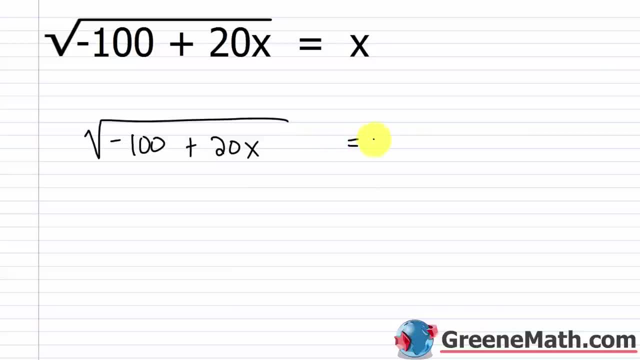 So negative: 100 plus 20x Is equal to x. I'm going to square this side and I'm going to square this side. So this is going to cancel with this and I'll just have this. I'll have negative. 100 plus 20x is equal to x squared. 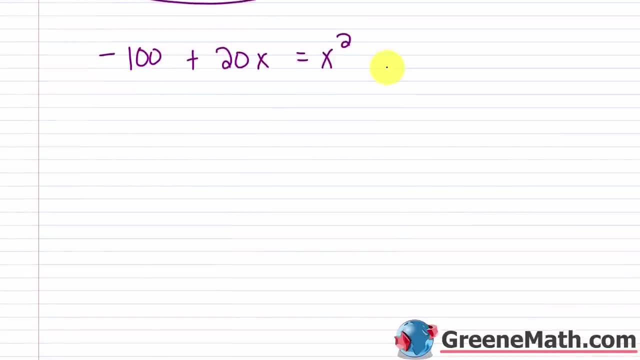 Again, I'm going to set this up by just putting everything on one side and setting it equal to 0. So let me add, Let me add 100 to both sides And let me subtract 20x away from each side, So that's going to be gone and be equal to 0. 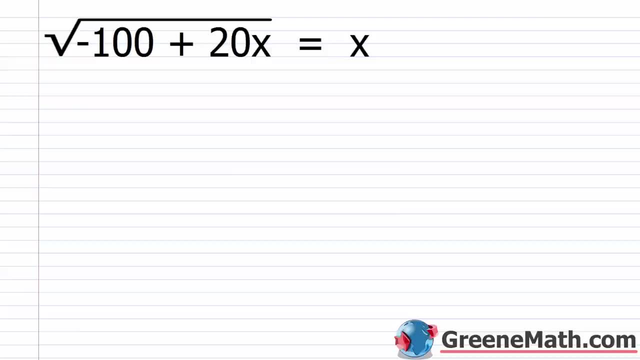 of negative 100 plus 20x, is equal to x. This is already isolated for us. So let's go ahead and just go into the step where we 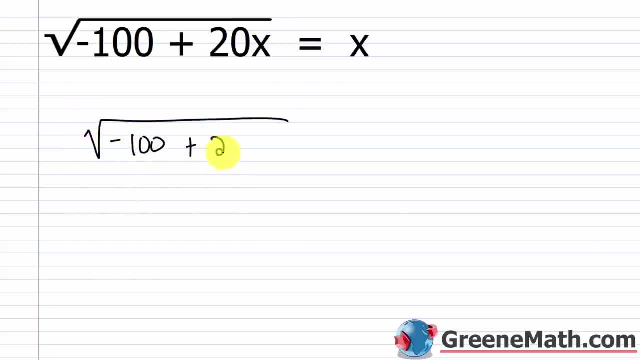 square both sides. So negative 100 plus 20x is equal to x, I'm going to square this side, and I'm going to square this side. So this is going to cancel with this and I'll just have this 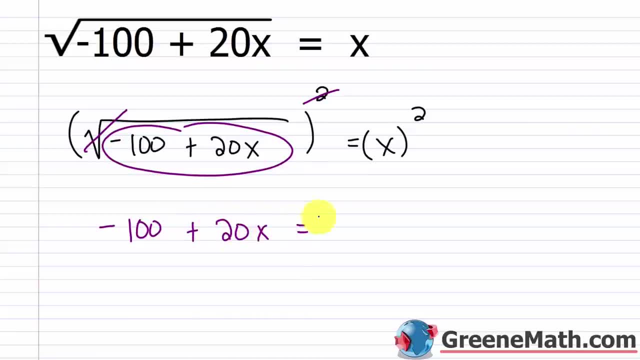 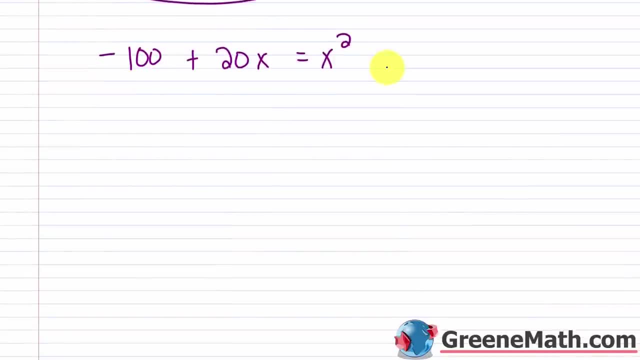 negative 100 plus 20x is equal to x squared. Again, I'm going to set this up by just putting everything on one side and setting it equal to zero. So let me add, let me add 100 to both sides. 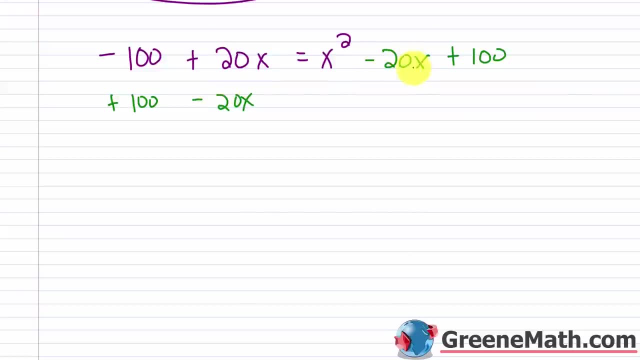 And let me subtract 20x away from each side. That's going to be gone and be equal to zero. And I like my zero to be on the right, and I like everything else to be on the left. So let's just rewrite it as x squared minus 20x plus 100 is equal to zero. 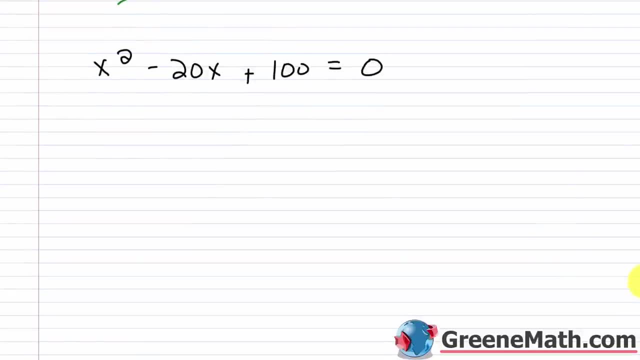 Okay, so now that that's set up, again, I gave you stuff that you could factor. So let's go ahead and factor this guy, we'll have x here and here, and then give me two integers, whose sum is negative 20, and whose product is 100. So we know that's going to be a negative and a negative, right, negative times negative is positive, negative plus negative is negative. So if I think about this, I could do negative 10 and negative 10, negative 10 and negative 10. 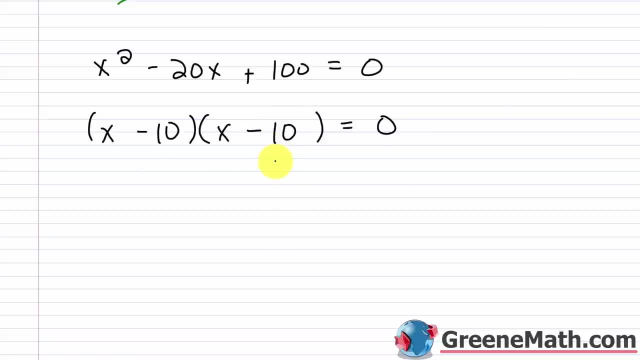 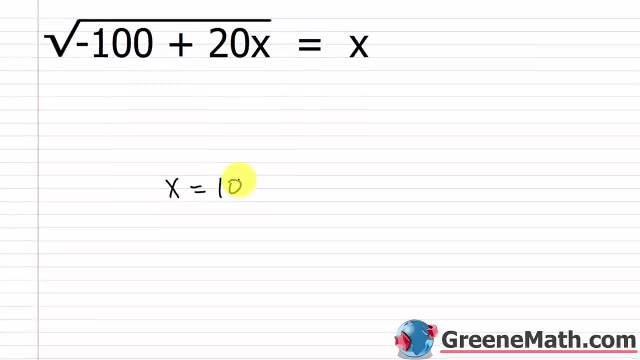 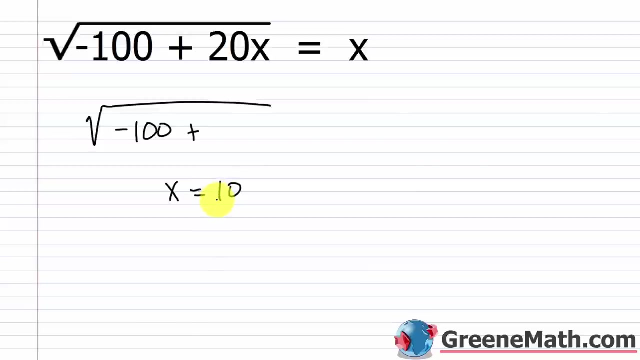 So that this would only have one solution, right, because it's basically x minus 10 as one factor, and x minus 10 is the other factor. So this would be one solution of x equals 10. So let's check this out in the original equation. Okay, so if I have square root of negative 100 plus 20 times 10, 20 times 10 is what? That's 200. This should equal 10. Let me kind of scooch this out of the way. 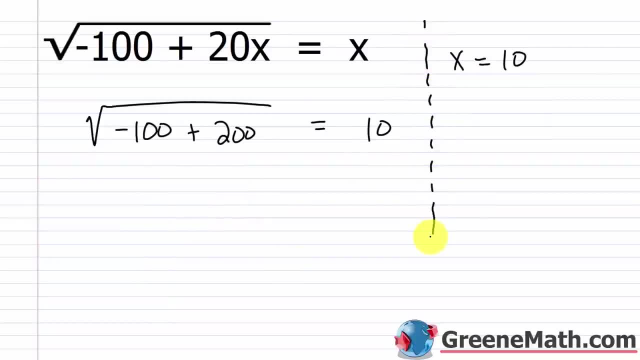 Okay, so if I simplify this, negative 100 plus 200 is 100. So I'd have the square root of 100 equals 10. And that's true, right? You get 10 equals 10. So yes, this is a valid solution, 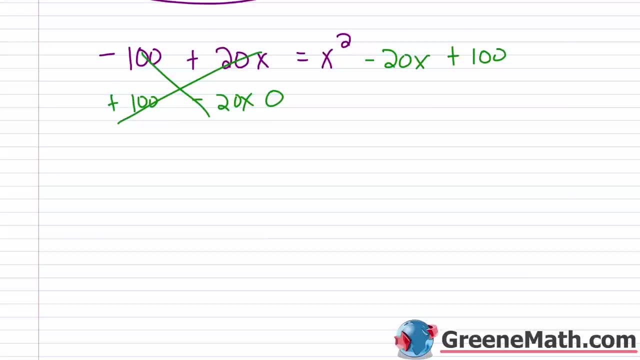 And I like my 0 to be on the right and I like everything else to be on the left. So let's just rewrite it as: x squared minus 20x plus 100 is equal to 0.. Okay, so now that that's set up. 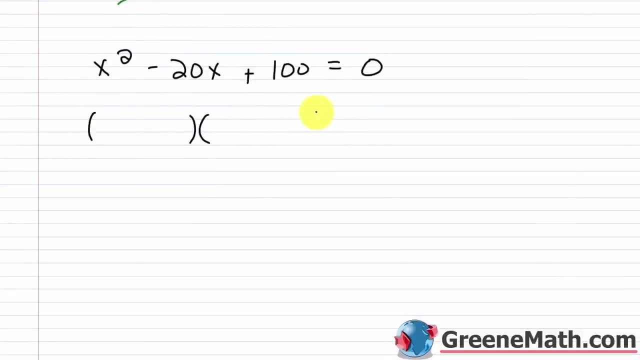 Again, I gave you stuff that you could factor, So let's go ahead and factor this guy. We'll have x here and here, And then give me Two integers whose sum is negative 20 and whose product is 100. So we know that's going to be a negative and a negative right, negative times. 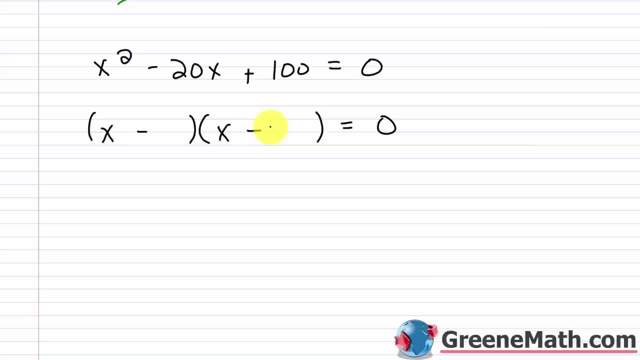 I give us positive, negative plus negative is negative. So if I think about this, I could do negative 10 and negative 10.. Negative 10 and negative 10.. I know that this would only have one solution right, Because it's basically x minus 10 as one factor and x minus 10 is the other factor. 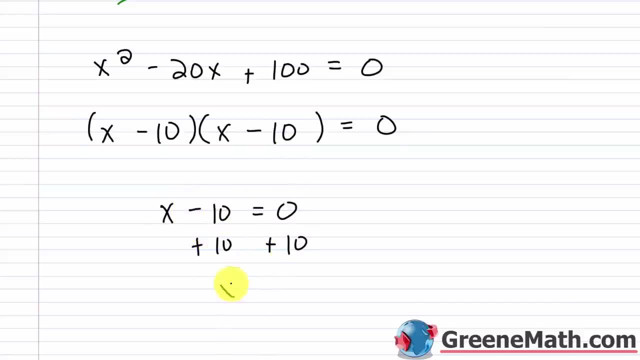 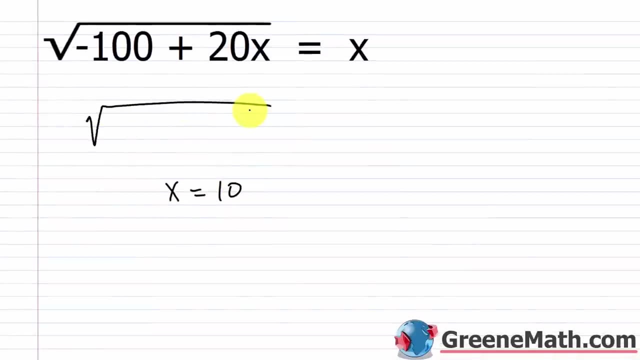 So this would be one solution Of x equals 10.. So let's check this out in the original equation. Okay, So if I have square root of negative, 100 plus 20 times 10, 20 times 10 is what, that's, 200.. 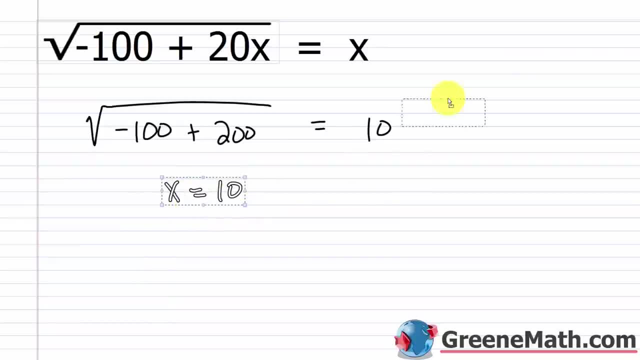 This should equal 10.. Let me kind of scooch this out of the way that over there. Okay, So if I simplify this, negative 100 plus 200 is a hundred. so I'd have the square root of a hundred equals 10, and that's true, right. 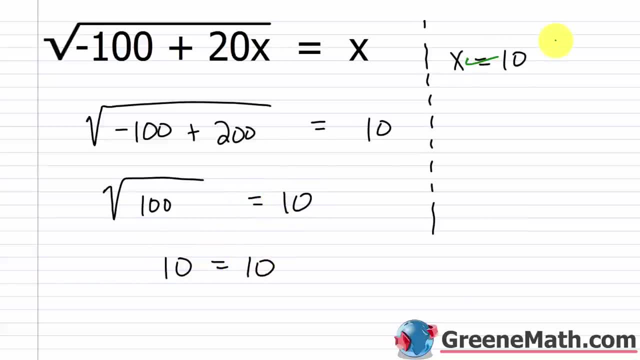 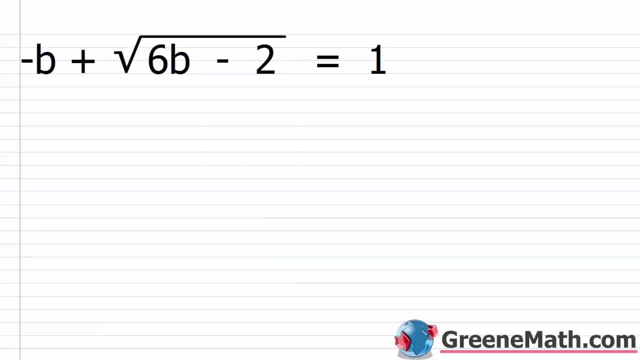 You get 10 equals 10.. So, yes, this is a valid solution: x equals 10.. All right, let's take a look at another one. So now we have negative B plus the square root of 6, B minus 2, and this equals 1.. 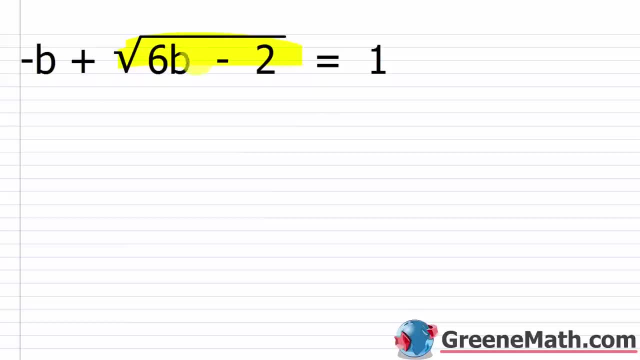 So notice how this is not isolated- Okay, the radical is not isolated. So we're getting into some more challenging problems, really just more tedious. So I can't just go ahead and start squaring things right. I can't square both sides. 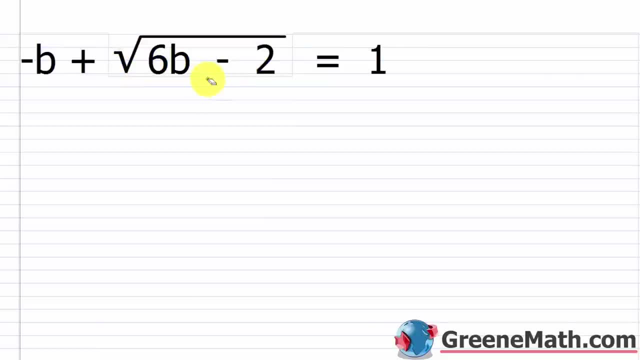 That's going to be really, really sloppy if I do that. So what I want to do again? I want to isolate the radical. So I'm just going to add B to both sides of the equation and I'm going to end up with the square root of 6. B minus 2 is equal to 1 plus B. 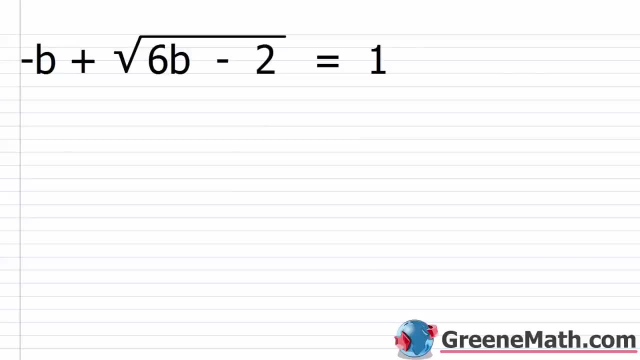 x equals 10. All right, let's take a look at another one. So now we have negative b plus the square root of 6b minus 2, and this equals 1. So notice how this is not isolated, okay? The radical is not isolated. So this is not isolated. So this is not isolated. So this is not isolated. 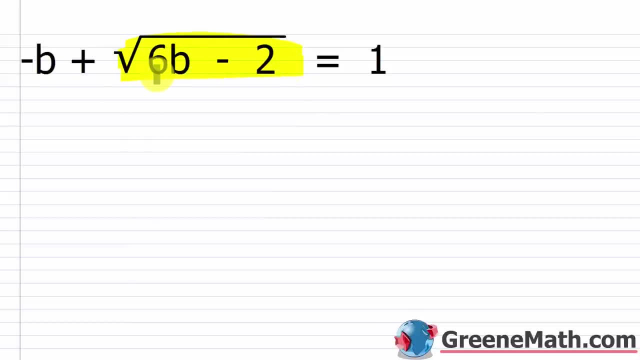 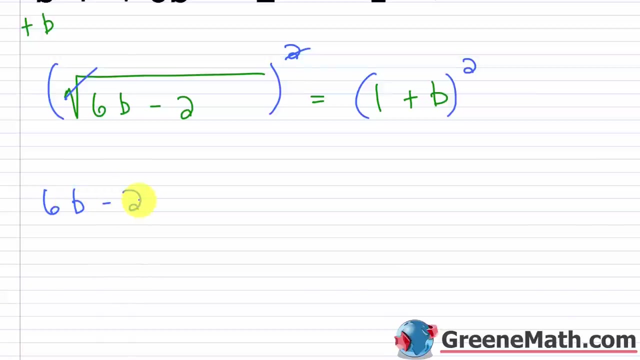 So we're getting into some more challenging problems, really just more tedious. So I can't just go ahead and start squaring things, right? I can't square both sides. That's going to be really, really sloppy if I do that. So what I want to do, again, I want to isolate the radical. So I'm just going to add b to both sides of the equation, and I'm going to end up with the square root of 6b minus 2 is equal to 1 plus b. Now, if I square both sides of the equation, I'm going to get rid of the radical. So this is going to cancel with this, and I'm going to have 6b minus 2. And remember, this has to be expanded. I can't do that common mistake where I just go, okay, 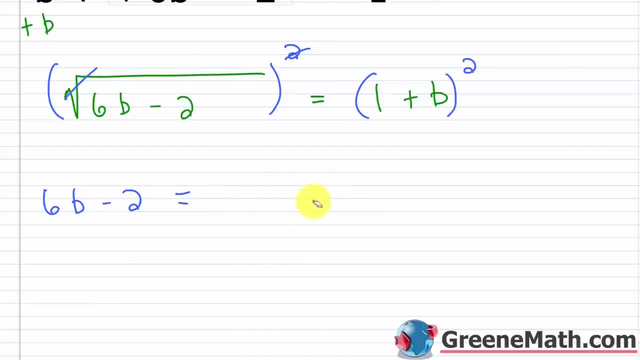 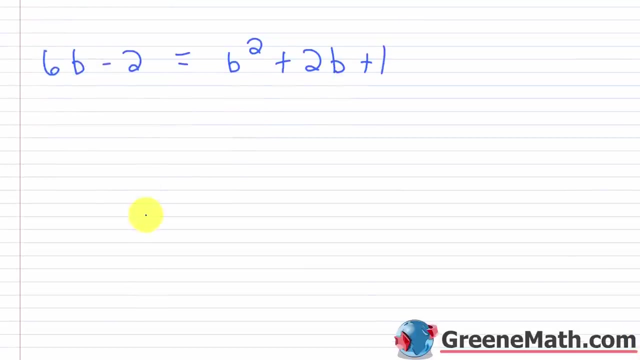 this is 1 squared plus b squared. We've covered that many, many times, and at this point in Algebra 1, you should realize this needs to be expanded. Now, fortunately for us, we know the formula for this to do it very quickly. It's this guy here, and this guy here. So we're going to b squared plus 2 times this guy times this guy plus this last guy squared. So really, it's b squared plus 2b plus 1. Let's rewrite that. b squared, b squared plus 2b plus 1. Let's scroll down a little bit. Get some room going. And let's add 2 to both sides of the equation. That's gone. 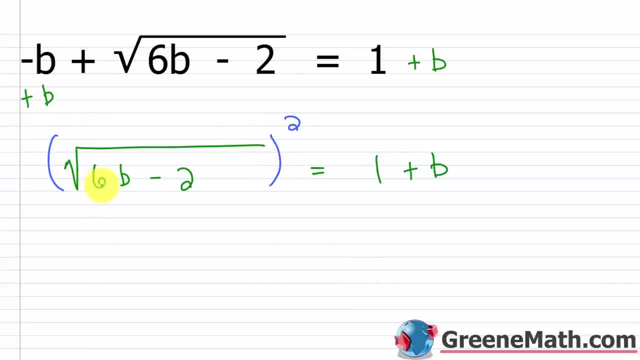 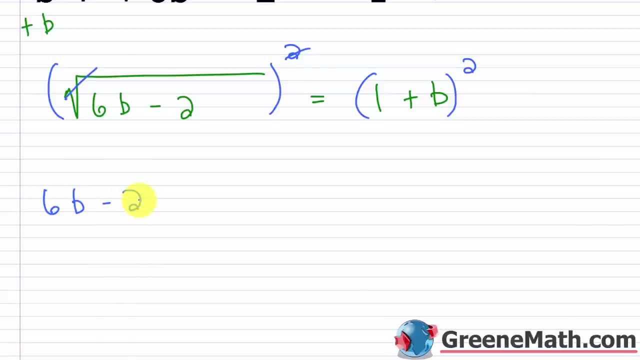 Now, if I square both sides of the equation, I'm going to get rid of the radical. So this is going to cancel with this and I'm going to have 6 B minus 2.. And remember, this has to be expanded. I can't do that common mistake where I just go. 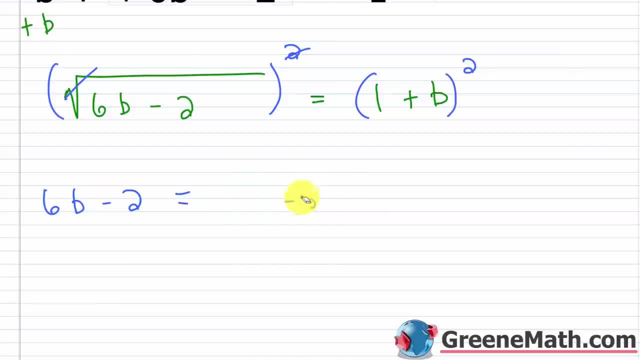 okay, this is 1 squared plus B squared. We've covered that many, many times and at this point in Algebra 1, you should realize this needs to be expanded Now. fortunately for us, we know the formula for this to do it very quickly. 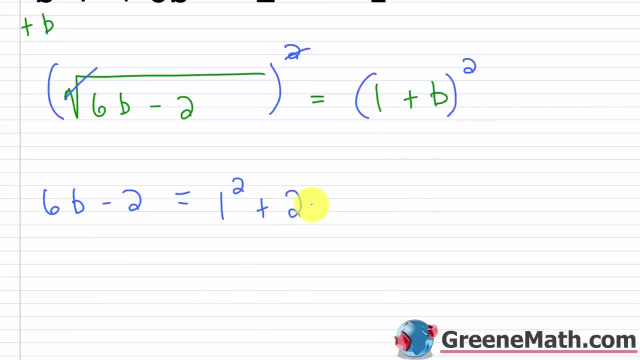 It's this guy squared plus 2 times this guy. times this guy plus this last guy squared, So really it's B squared plus 2B plus 1.. Let's rewrite that B squared: B squared plus 2B plus 1.. 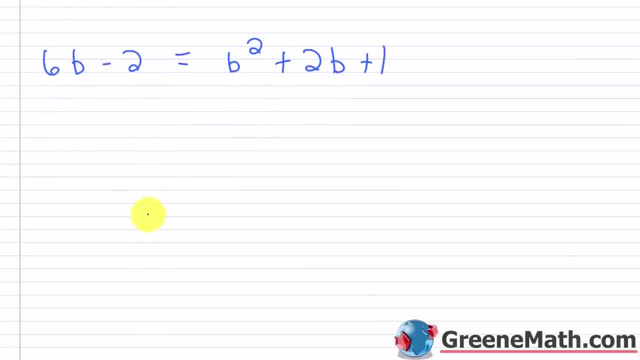 Let's scroll down a little bit, Get some room going And let's add 2 to both sides of the equation, That's gone. And let's subtract 6 B away from each side of the equation, So that's gone. So I would have 0 over here on the left is equal to. 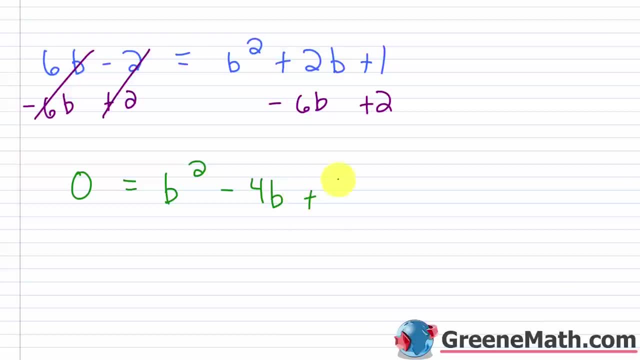 We have B squared minus 4B plus 3.. Now let me just kind of switch this around and say: okay, I have B squared minus 4B plus 3 equals 0.. Again, that's just personal preference. You don't have to do that. 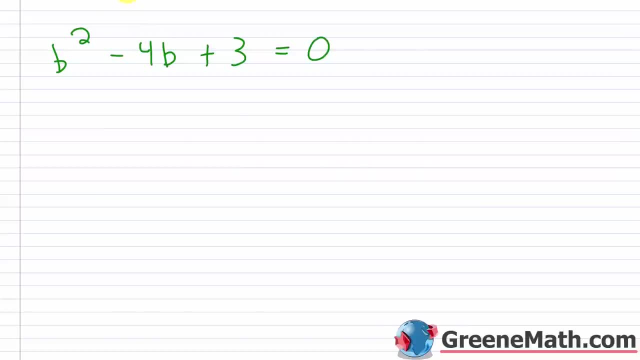 It's just up to you, Okay. so now what I want to do is factor the left side. So this is going to be factored and equal to 0. And I know the first terms would be B and B. So now I need to find two integers whose sum is negative 4 and whose product is 3.. 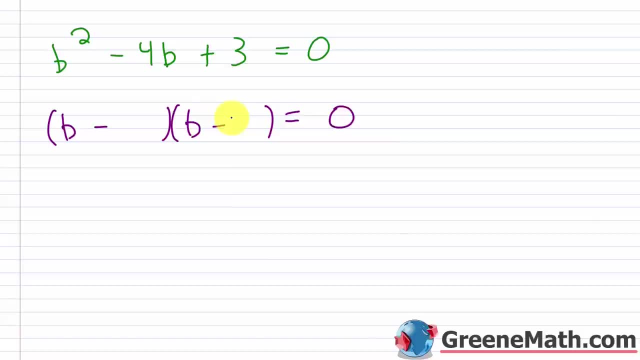 So I know this has to be a negative and a negative. right, Because negative times negative is positive. Negative plus negative is negative. It's easy, because 3 is a prime number. right, It's only 1 times 3.. So it has to be 3 and 1, right. 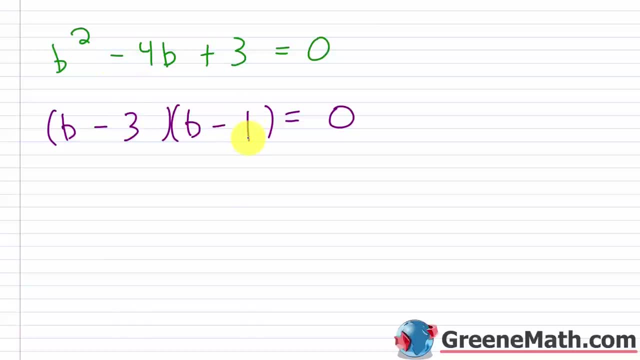 So B minus 3, that quantity, times B minus 1, that quantity. So to solve this again, use the zero product property. We're going to set each factor With a variable equal to 0. So we'd have B minus 3 equals 0 or B minus 1 equals 0. 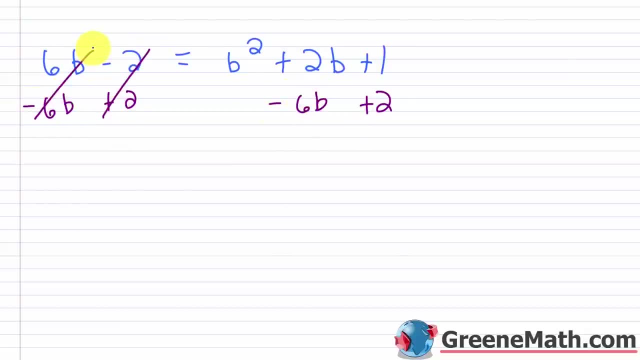 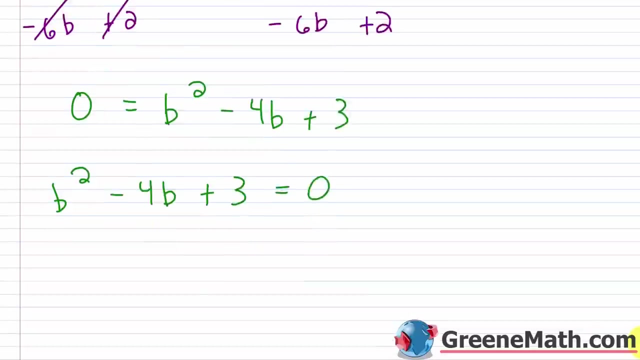 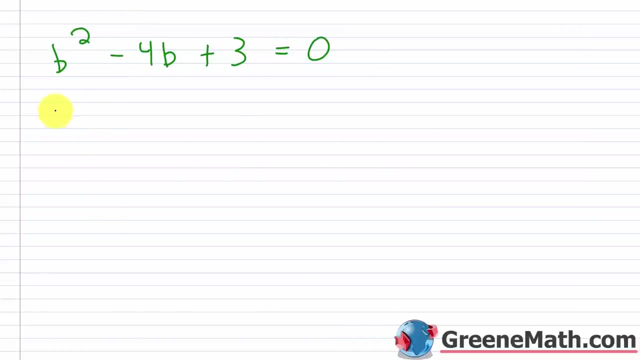 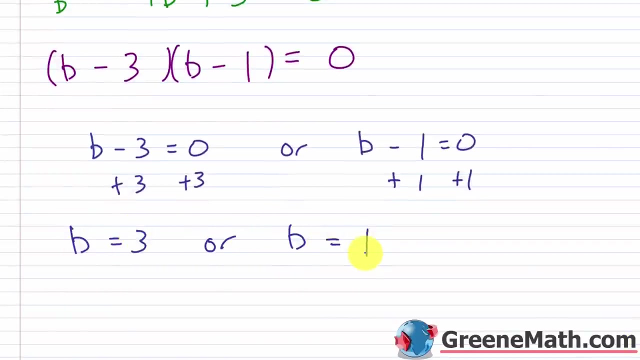 And let's subtract 6b away from each side of the equation. So that's gone. So I would have 0 over here on the left is equal to, we have b squared minus 4b plus 3. And let me just kind of switch this around and say, okay, I have b squared minus 4b plus 3 equals 0. Again, that's just personal preference. You don't have to do that. It's just up to you. Okay, so now what I want to do is factor the left side. So this is going to be factored and equal to 0. And I know the first terms would be b and b. So now I need to find two integers whose sum is negative 4 and whose product is 3. So I know this has to be a negative and a negative, right? Because negative times negative is positive. Negative plus negative is negative. It's easy because 3 is a prime number, right? It's only 1 times 3. So it has to be 3 and 1, right? So b minus 3, that quantity, times b minus 1, that quantity. So to solve this, again, use the 0 product property. We're going to set each factor with a variable equal to 0. So we'd have b minus 3 equals 0 or b minus 1 equals 0. We'd add 3 to each side of the equation here. We'd add 1 to each side of the equation here. And what we're going to end up with is b is equal to 3 or b is equal to 1. All right, so let's check this. 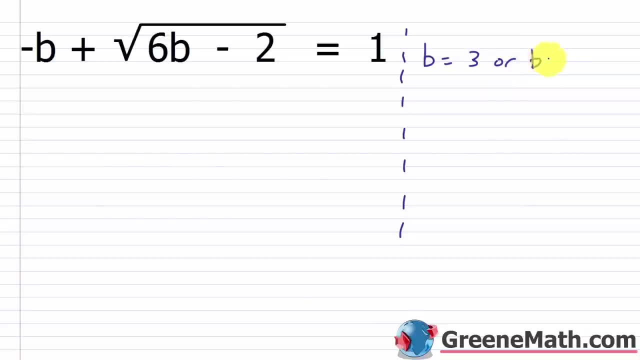 And we had b is equal to 3 or b is equal to 1. All right, so let's start out with b equals 3. So let's plug in a 3 here and here and see if we get a true statement. So we would have negative 3 plus the square root of 6 times 3 is 18 minus 2. So we know we can just replace that with 16. And this should be equal to 1. Square root of 16 is 4. So I'd have negative 3 plus 4. That is 1. You get 1 equals 1. So yes, this is a valid solution. All right, for the next one, I'd replace my b with a 1. So I'd have negative 1 plus the square root of 6 times 1, which is 6, minus 2, which would give me 4. So the square root of 4. And this should be equal to 1. Now, the square root of 4 is 2. So I'd have negative 1 plus 2. That gives me 1. And that equals 1. 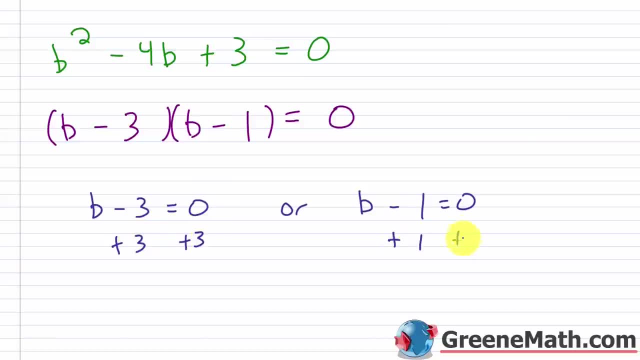 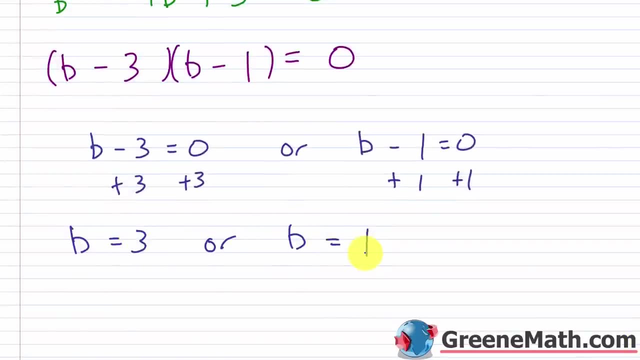 We'd add 3 each side of the equation here, We'd add 1 each side of the equation here, And what we're going to end up with is B is equal to 3 or B is equal to 1.. All right, 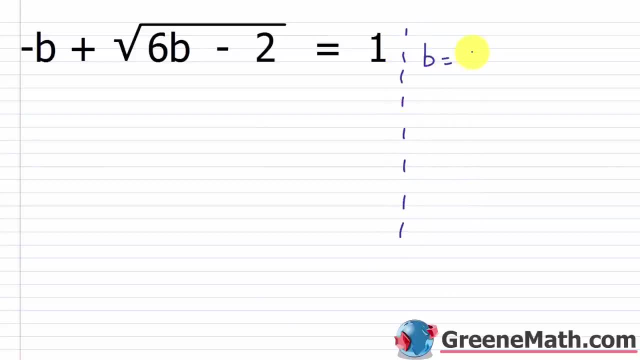 So let's check this. and we had: B is equal to 3 or B is equal to 1.. All right, So let's start out with B equals 3.. So let's plug in a 3.. Let's see here and here and see if we get a true statement. 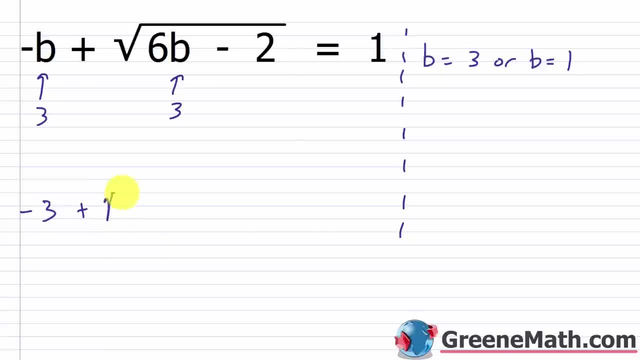 So we would have negative 3 plus the square root of 6 times 3 is 18 minus 2.. So we know we can just replace that with 16 and this should be equal to 1.. Square root of 16 is 4.. 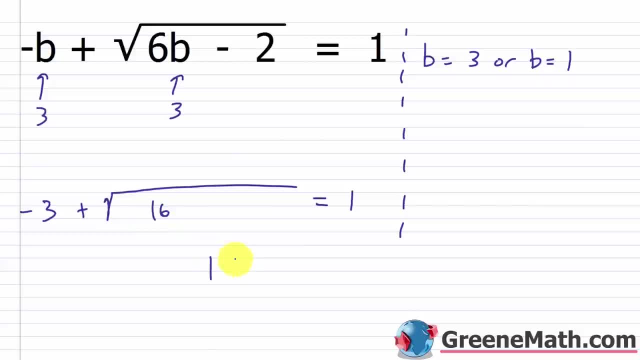 So I'd have negative 3 plus 4. That is 1. You get 1 equals 1.. So, yes, this is a valid solution. All right, For the next one, I'd replace my B with a 1.. 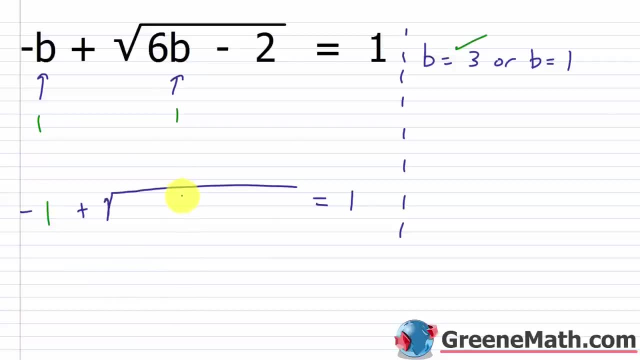 So I'd have negative 1 plus the square root of 6 times 1, which is 6 minus 2, which would give me 4.. So the square root of 4 and this should be equal to 1.. Now the square root of 4 is 2.. 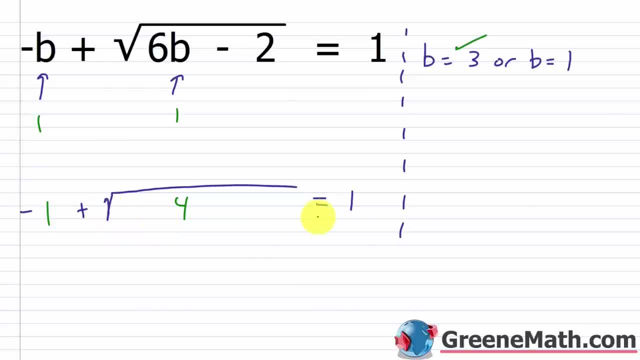 So I'd have negative 1 plus 2. That gives me 1 and that equals 1. So we get 1 equals 1.. Again, this solution is valid: B equals 1. So we have B equals 3 here or B equals 1.. 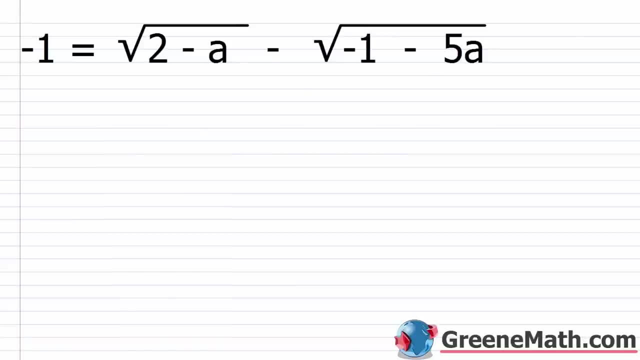 Okay, For the last problem that we're going to look at in this lesson, we're going to dive into something that's much more tedious. This is a type of problem where you want to focus as much as you can, because it's very, very easy in these longer problems to make a silly mistake that costs you the right answer in the end, right? 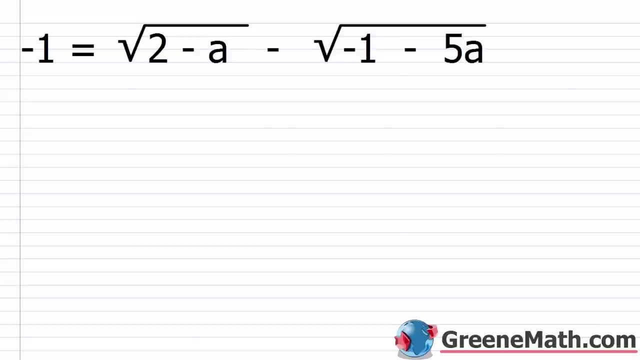 The worst thing is you do all this work, You made some silly mistake. and then you go to check your answer and you're like: ah, you know I made a mistake and you have to start the problem over. So just pay close attention. 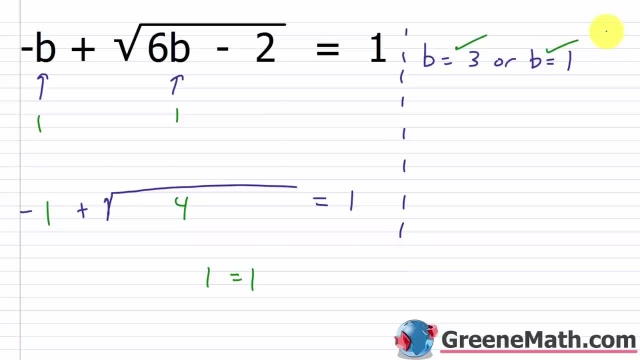 So we get 1 equals 1. Again, this solution is valid. b equals 1. So we have b equals 3 here 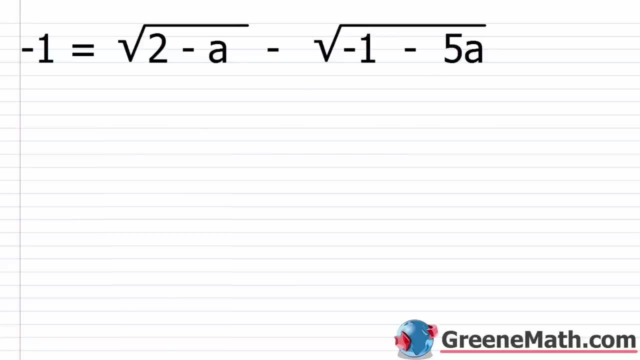 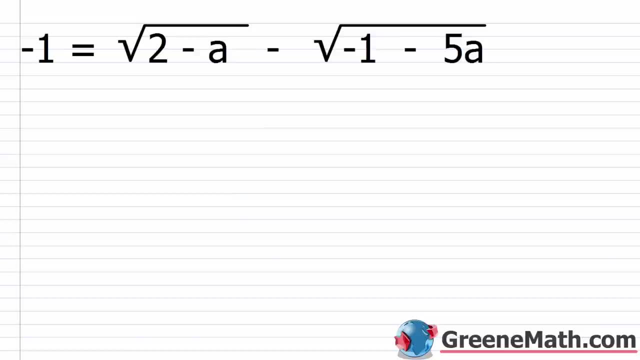 And you have to start the problem over. So just pay close attention to the ones like this that are very, very tedious. Okay, so we have negative 1 is equal to the square root of 2 minus a minus the square root of negative 1 minus 5a. Now, up until this point, we've seen that we would square both sides after we isolated the radical and we were radical free. 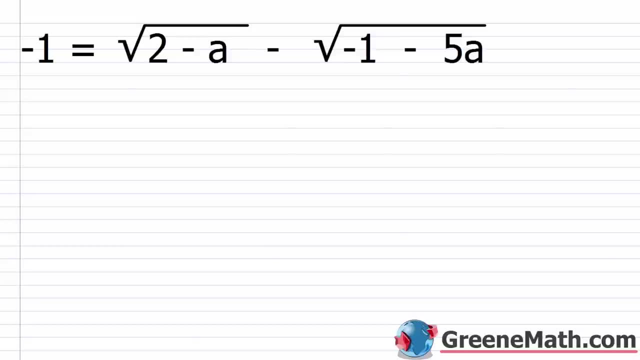 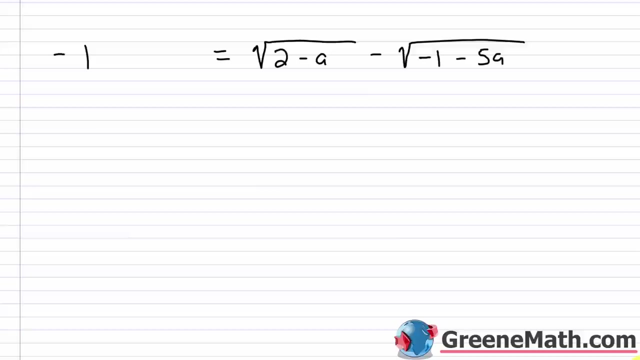 In this case, we have two radicals involved. So that's not going to happen. What we have to do is isolate one radical at a time, okay, and work our way through the problem. So that's what makes this much more tedious. So let's just copy the problem. So negative 1 is equal to the square root of 2 minus a minus the square root of negative 1 minus 5a. Now, I want to isolate one of these guys. It doesn't matter which one I choose. I'm going to put the same answer in the end. I think it would be easier for me to isolate this guy right here. And so I'm going to add the square root of negative 1 minus 5a to both sides. So over here, it's going to cancel itself and go away. And I'm just going to add it over here. So plus the square root of negative 1 minus 5a. Now, what I can do at this point is I can square 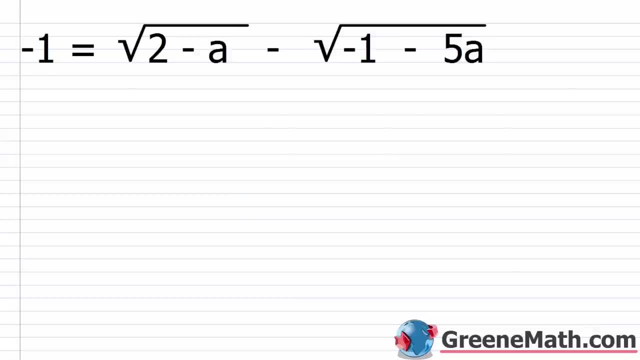 Pay close attention to the ones like this that are very, very tedious. Okay, So we have: negative 1 is equal to the square root of 2 minus a, minus the square root of negative 1 minus 5a. Now, up until this point, we've seen that we would square both sides after we isolated the radical and we were radical free. 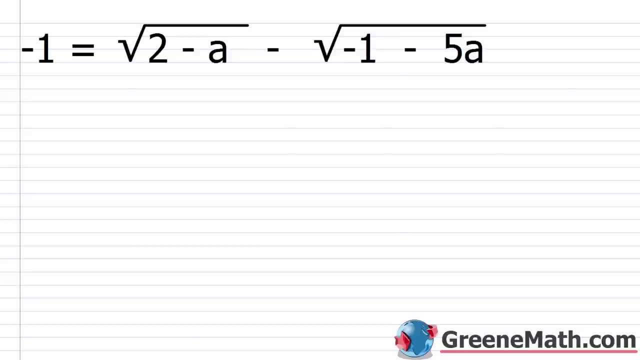 In this case, we have two radicals involved, So that's not going to happen. What we have to do is isolate one radical at a time, Okay, And work our way through the problem. So that's what makes this much more tedious. 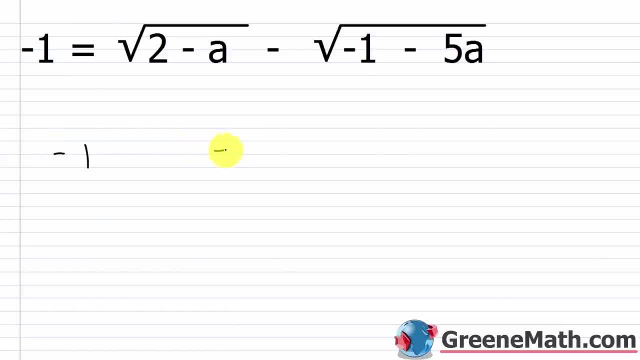 So let's just copy the problem. So negative 1 is equal to the square root of 2 minus a, minus the square root of negative 1 minus 5a. Now I want to isolate one of these guys. It doesn't matter which one I choose. 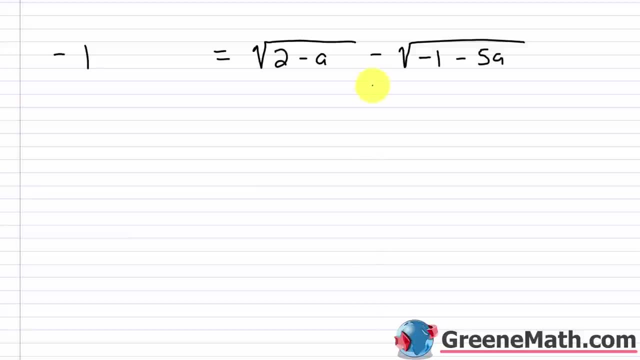 I'm going to put the same answer. in the end, I think it would be easier for me to isolate this guy right here, And so I'm going to add the square root, The square root of negative 1 minus 5a, to both sides. 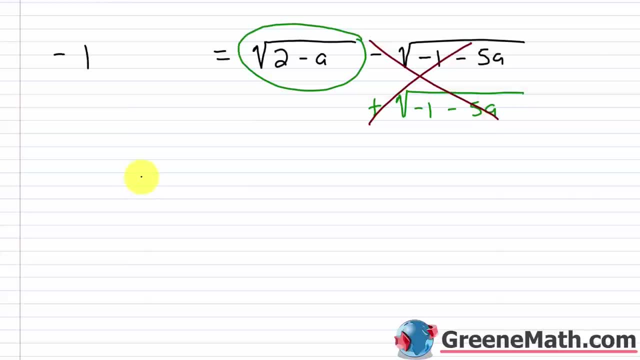 So over here it's going to cancel itself and go away, And I'm just going to add it over here. So, plus the square root of negative 1 minus 5a. Now, what I can do at this point is I can square both sides of the equation and I'll get rid of one and only one of the radicals. 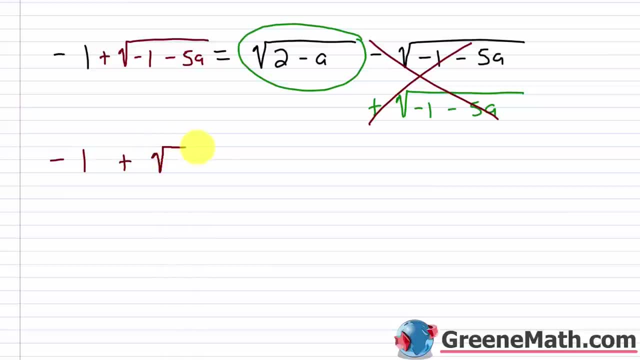 So I have negative 1 plus the square root of Negative 1 minus 5a. I'm going to square this guy. And then this is equal to: We have the square root of 2 minus a, and I'm going to square this guy. 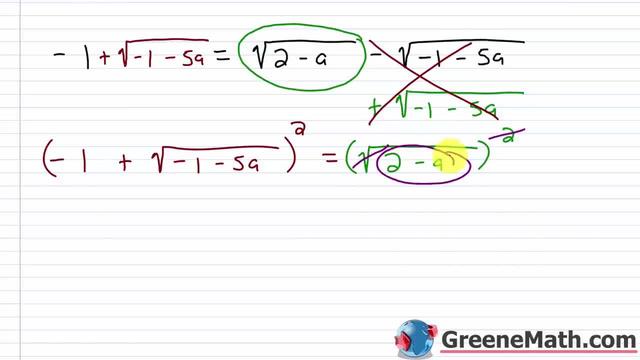 Now we know at this point that this would cancel with this and I'm left with this, So I'm going to put equals 2 minus a over here for this side. It looks like it would be kind of complex to do that, But again we can use our special products formulas. 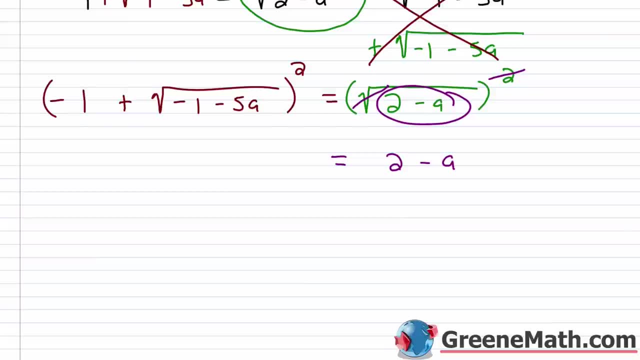 To speed up the process. That's why we went through and memorize those. So I know for this I would square the first guy. Negative 1 squared is positive 1. So let's write that all the way down here. And then the next thing would be we would have plus 2 times this guy. times this guy. 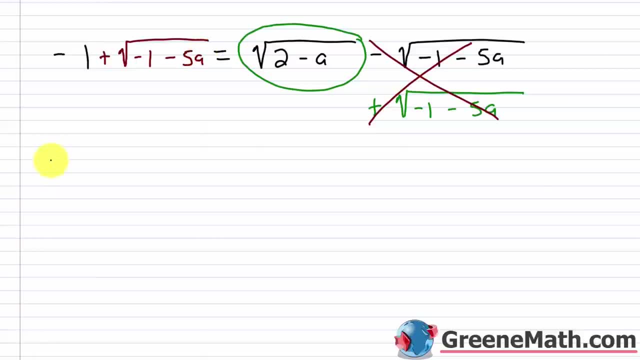 one and only one of the radicals. So I'll have negative 1 plus the square root of negative 1 minus 5a. And I'm going to square this guy. And then this is equal to, we have the square root of 2 minus a. And I'm going to square this guy. Now, we know at this point that this would cancel with this. And I'm left with this. So I'm going to put equals 2 minus a over here. 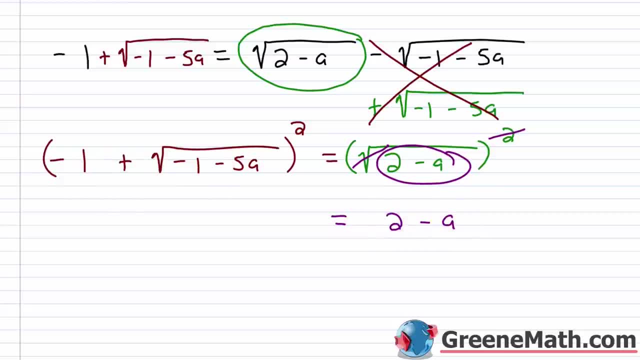 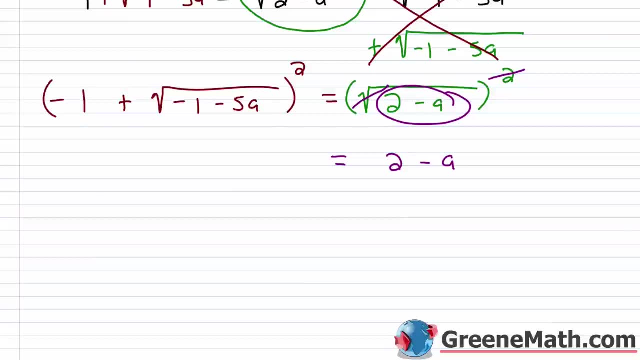 For this side, it looks like it would be kind of complex to do that. But again, we can use our special products formulas to speed up the process here. That's why we went through and memorized those. So I know for this, I would square the first guy. Negative 1 squared is positive 1. So let's write that all the way down here. And then the next thing would be, we would have plus 2 times this guy times this guy. 2 times negative 1 is negative 2. So I'll write minus 2. Then times the square root of... Negative 1 minus 5a. Then the last thing is I want this guy squared. Well, if I squared the square root of negative 1 minus 5a, we, again, know that this would cancel with this. And I'd be left with this. So I'd have minus 1 minus 5a. All right. So now that that's worked out, 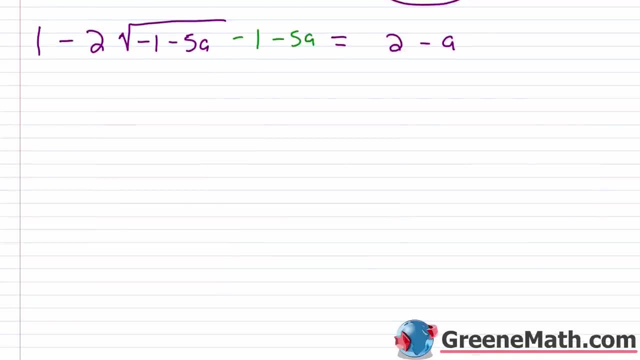 what I want to do at this point is simplify. So when I look across, I see that I have a 1 and a negative 1. So those would cancel. And then I see that I have a negative 5a and a negative a. So I can add 5a to both sides of the equation. That's going to cancel. So I'm going to have this negative 2 times the square root of negative 1 minus 5a. 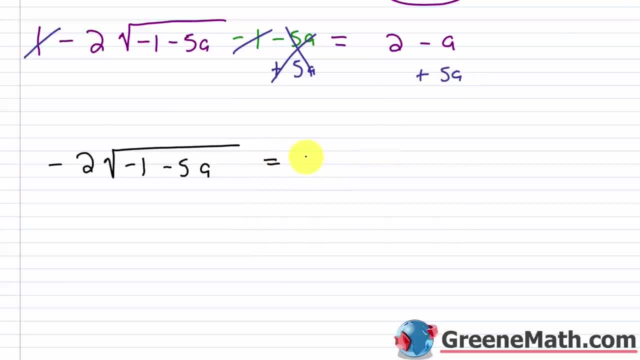 And this is equal to... And I'm just going to reorder this to 4a plus 2. 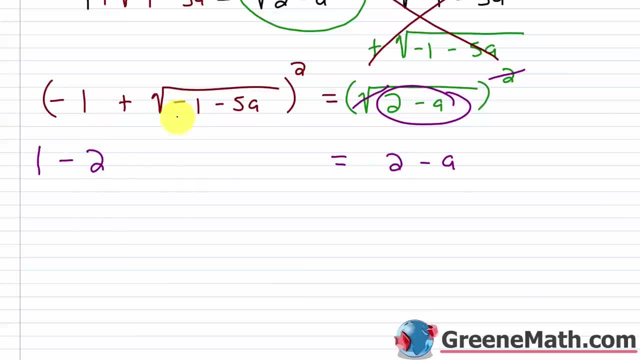 2 times negative. 1 is negative 2.. So I'll write minus 2.. Then times the square root of negative 1 minus 5a. Then the last thing is: I want this guy squared. Well, if I squared The square root of negative 1 minus 5a. 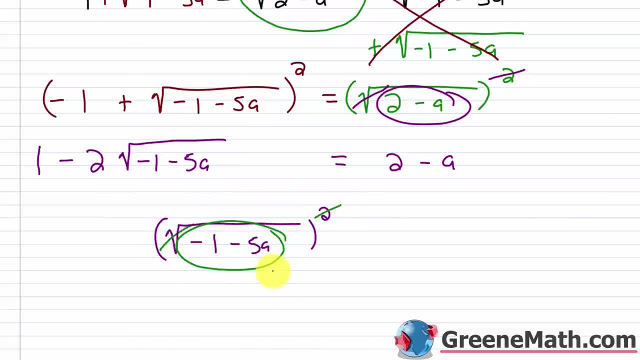 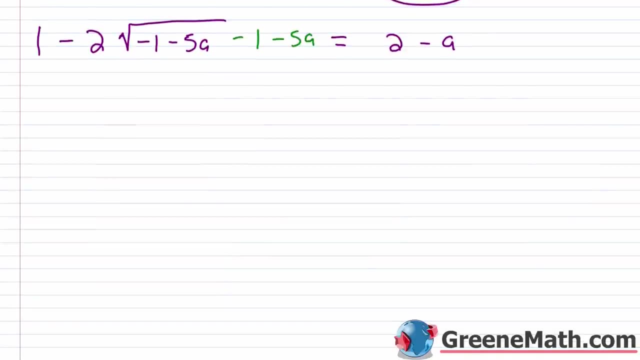 We again know that this would cancel with this and I'd be left with this, So I'd have minus 1, minus 5a, All right. So now that that's worked out, what I want to do with this point is simplify. So when I look across, I see that I have a 1 and a negative 1.. 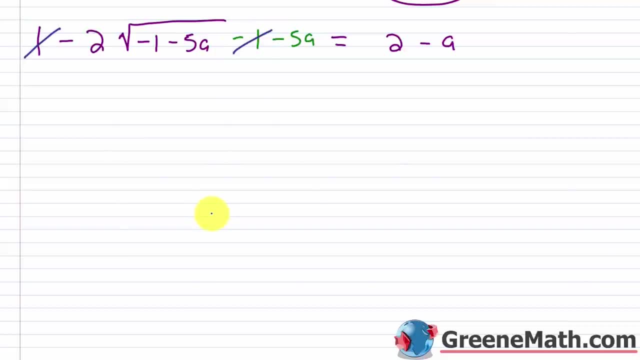 So those would cancel. and then I see that I have a negative 5a And a negative a, so I can add 5a to both sides of the equation. That's going to cancel. So I'm going to have this negative 2 times the square root of negative, 1 minus 5a. 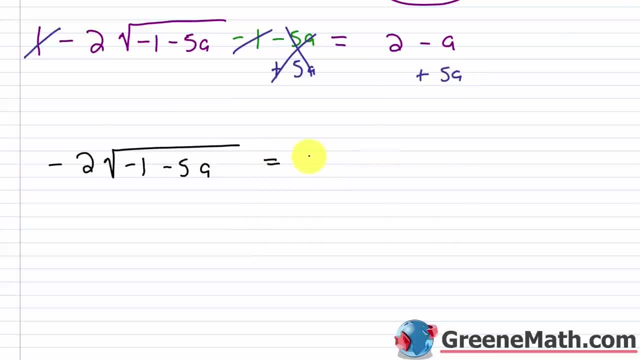 And this is equal to- and I'm just going to reorder this to: 4a plus 2.. Okay, negative a plus 5a is 4.. Now what I want to do is I want to square both sides of this equation. 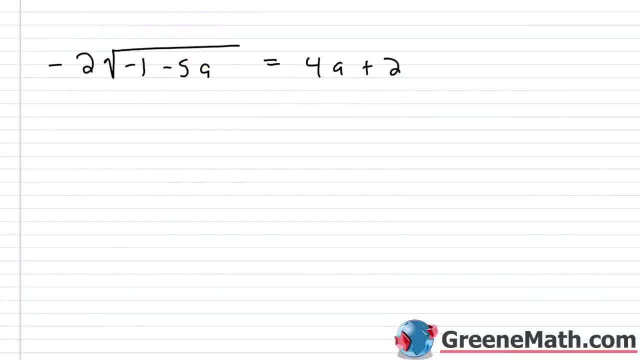 One more time to get rid of this radical. This is going to be a little bit tricky and I'm going to explain why. So let me square this side and let me square this side Now. when I square this guy, I want you to think back to when I squared something like a times b squared. 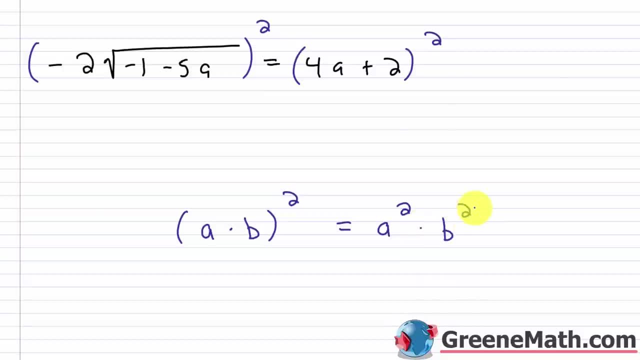 This is equal to a squared times b squared right. We all should agree on that. If I look at this more closely, This is really what this is: negative 2. Times this quantity- Let me just put it in parentheses- negative 1 minus 5a. 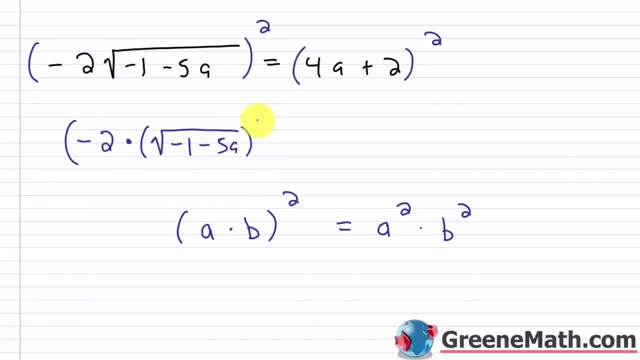 Okay, so if I squared this, if I squared this, I would end up with what? let me kind of erase this, Following that model, and have negative 2 squared times, This square root of negative 1 minus 5a that guy squared now. 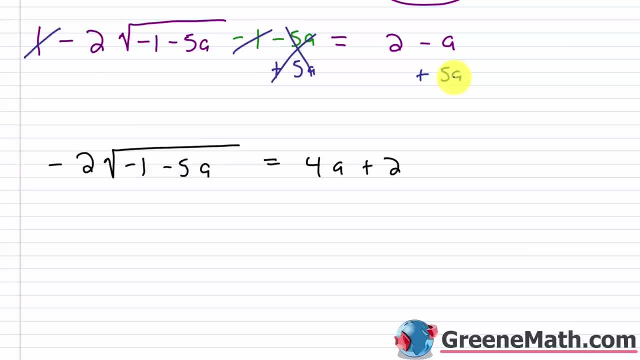 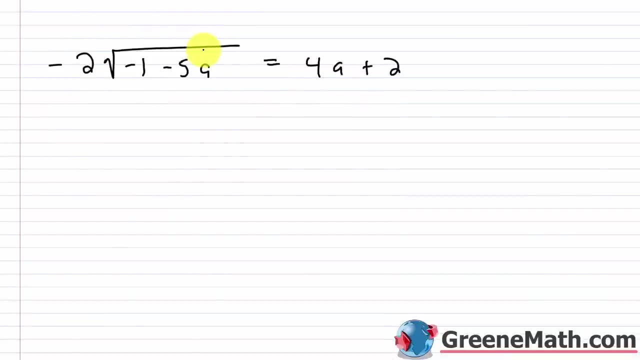 Okay. Negative a plus 5a is 4. Now, what I want to do is I want to square both sides of this equation one more time to get rid of this radical. This is going to be a little bit tricky, and I'm going to explain why. So let me square this side, and let me square this side. Now, when I square this guy, I want you to think back to when I squared something like a times b squared. This is equal to a squared times b squared. All right. We all should agree on that. If I look at this more closely, this is really what? This is negative 2 times this quantity. Let me just put it in parentheses. Negative 1 minus 5a. Okay. 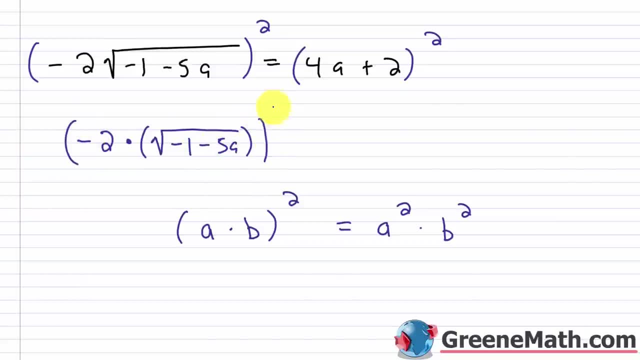 So if I squared this, if I squared this, I would end up with what? Let me kind of erase this. 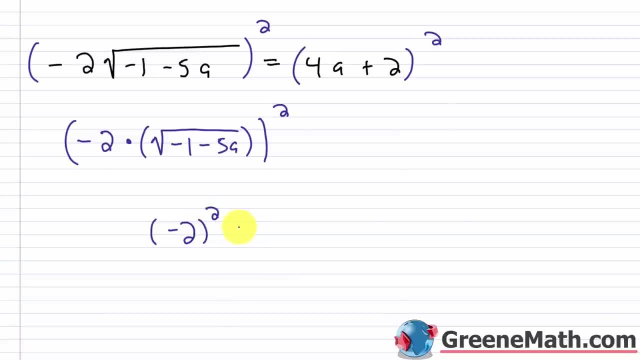 Following that model, I'd have negative 2 squared times this square root of negative 1 minus 5a, that guy squared. Now, this will cancel with this and give me this. Where students make a mistake is you're still multiplying here. So let me kind of go through this. Let me move this down, or I'll actually move it over to get some room. And let me show you what I mean. So when this comes down, negative 2 squared, which I have here, would be positive 4. But this is still multiplying the result of this. So the result of this is the quantity negative 1 minus 5a. Okay. 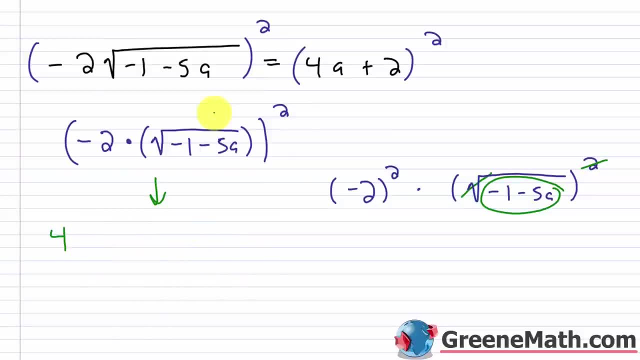 The common mistake that you see is, let me just erase this. Students just go, okay, well, this is 4 minus 1 minus 5a. That's not correct. Again, if we go back to the example of a times b, and this is squared, we all should agree that this is a squared times b squared. Okay. 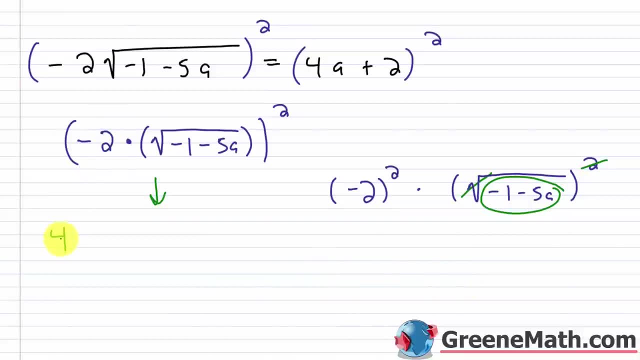 So it's the same thing here. This is squared, that's 4, times the result of this squared, which is the quantity negative 1 minus 5a. So you've got to make sure that you do that correctly. 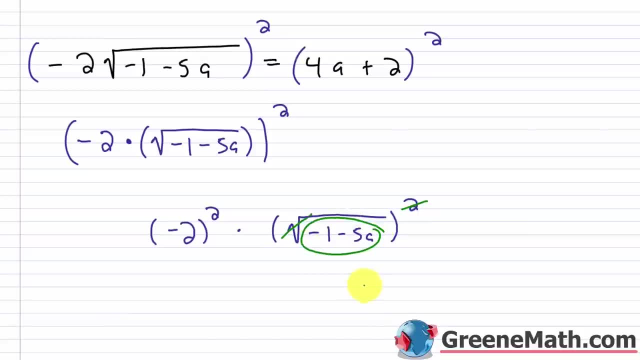 This will cancel with this and give me this: Where students make a mistake, is you still multiplying here? So let me kind of go through this. Let me, let me move this down, Or I'll actually move it over to get some room- and let me show you what I mean. 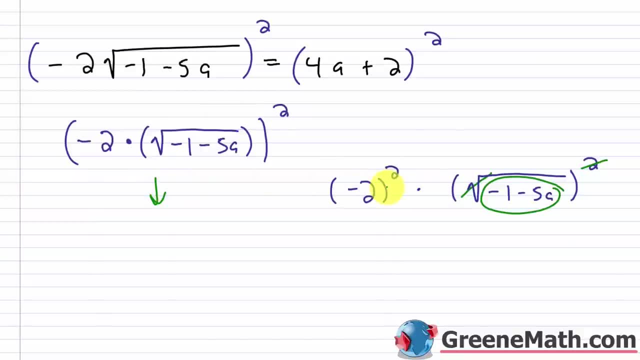 So, when this comes down, negative 2 squared, which I have here, would be positive 4. But this is still multiplying the result of this. So the result of this is the quantity negative 1 minus 5a. So the result of this is the quantity negative 1 minus 5a. 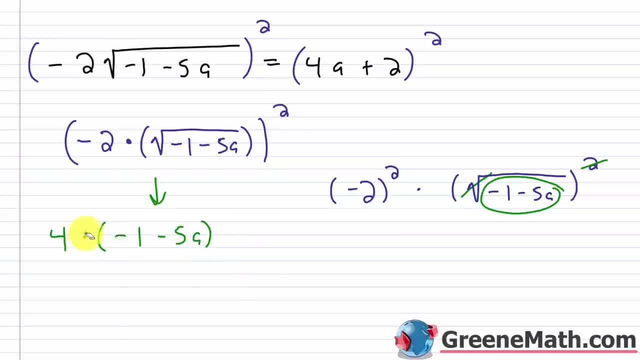 Okay. the common mistake that you see is: let me just erase this soon, Just go. Okay. Well, this is 4 minus 1 minus 5a. That's not correct. again, If we go back to the example of a times B, and this is squared: 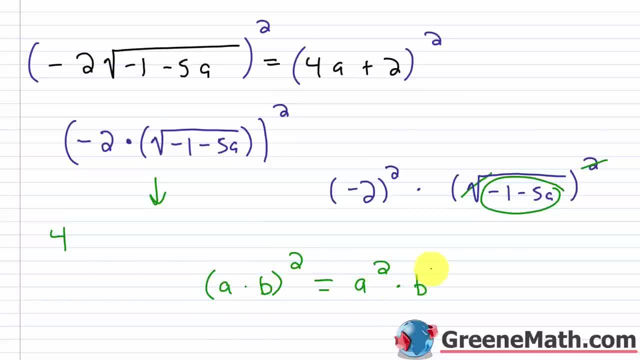 We all should agree that this is a squared times B squared. Okay, so it's the same thing here. This is squared. That's 4 times the result of this squared, Which is The quantity negative: 1 minus 5a. 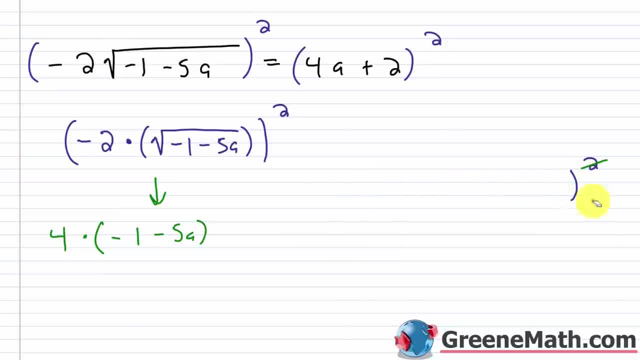 So you've got to make sure that you do that correctly, All right. So with that being said, let's put: this is equal to: We have 4a plus 2, that quantity squared, And again we can use our special products formulas for this. 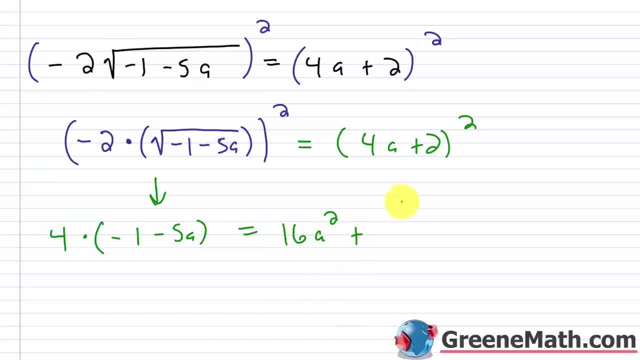 Square the first guy, That's 16a, squared plus 2 times this guy. times this guy 2 times 4 is 8.. 8 times 2 is 16.. Then times a, Then plus The last guy squared. 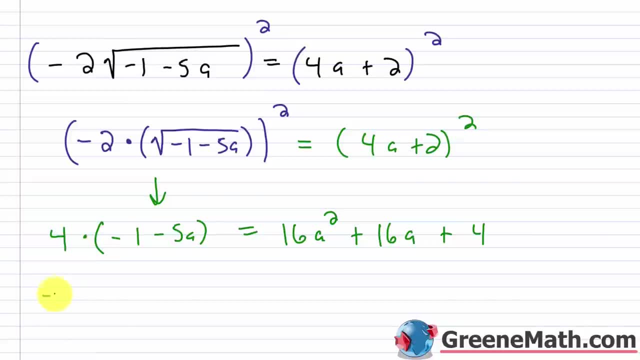 All right. So simplifying here on the left, 4 times negative 1 is negative 4.. And then 4 times negative 5a is negative 20a. So this equals 16a squared plus 16a plus 4.. 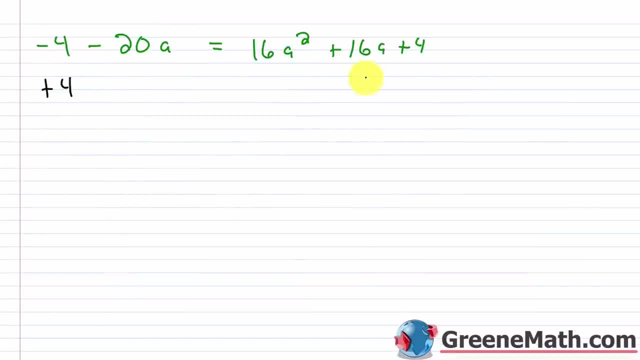 Let me scroll down, And so let me add 4 to both sides of the equation. here Let me add 28 of both sides of the equation, So this would be 0. So I'd have: 0 is equal to 16a squared. 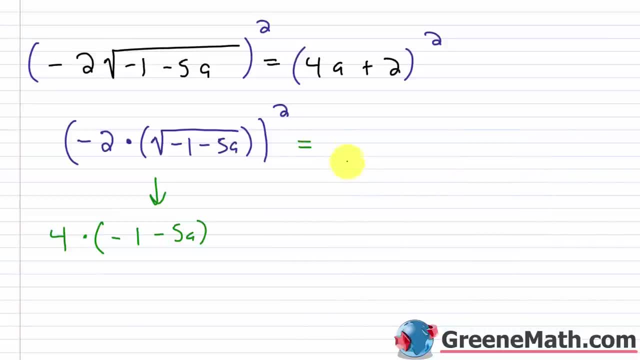 All right. So with that being said, let's put this is equal to, we have 4a plus 2, that quantity squared. And again, we can use our special products formulas for this. Square the first guy, that's 16a squared. Plus 2 times this guy times this guy. 2 times 4 is 8. 8 times 2 is 16. Then times a. Then plus the last guy squared. All right. So, simplifying here on the left, 4 times negative 1 is negative 4. And then 4 times negative 5a is negative 20a. So this equals 16a squared plus 16a plus 4. Let me scroll down. And so let me add 4 to both sides of the equation here. 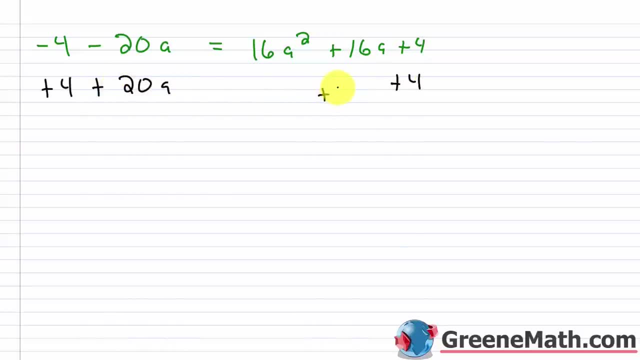 And let me add 20a to both sides of the equation. So this would be 0. 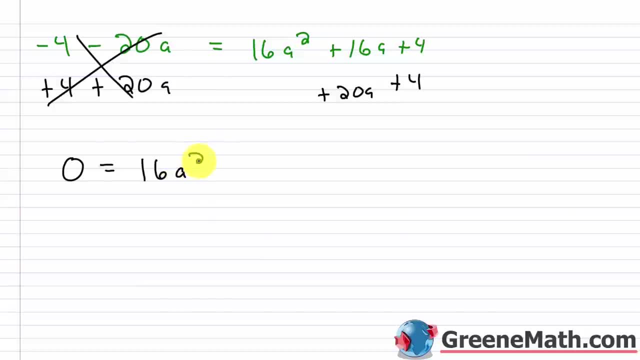 So I'd have 0 is equal to 16a squared, 16a plus 20a is 36a, so plus 36a, and then plus 8. 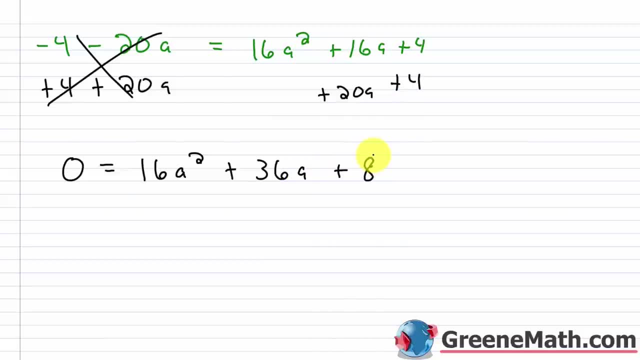 And again, I like the 0 on the right side. It doesn't matter. It's just personal preference. 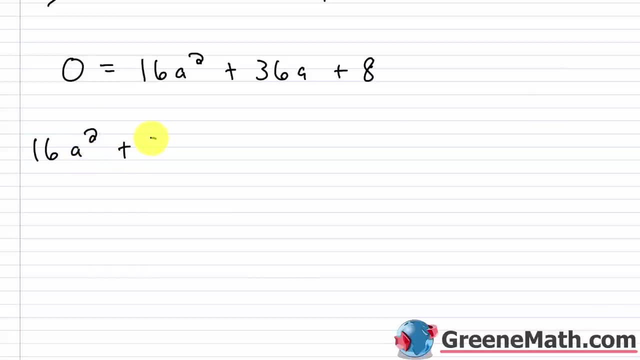 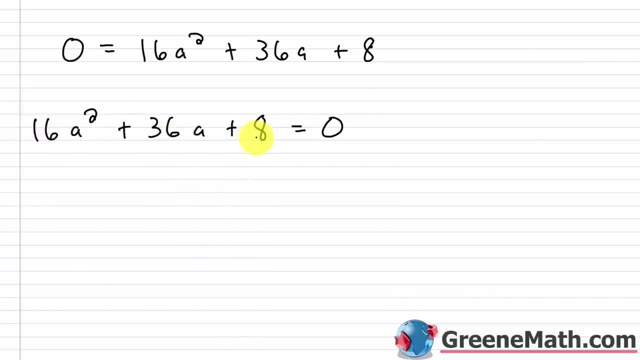 So I'm going to rewrite this as 16a squared plus 36a plus 8 equals 0. So before I move forward, I notice that I can pull a 4 out of everything. 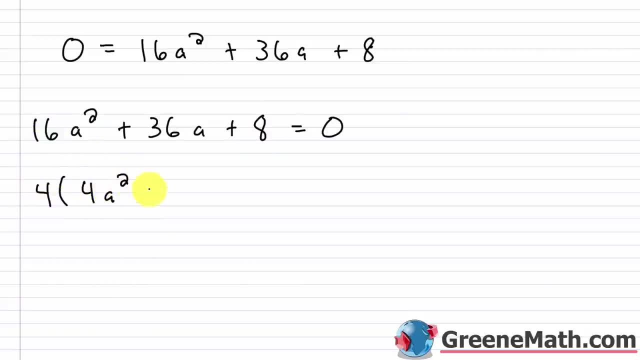 So if I pull a 4 out, this would be 4a squared plus 9a plus 2, and this is equal to 0. 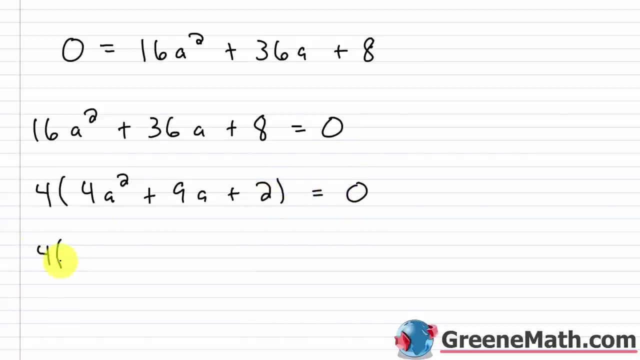 So to factor the inside here, I'm going to use factoring by grouping. So give me two integers whose product... ...whose product... ...whose product is 8 and whose sum is 9. That's easy. That's 8 and 1. So let's rewrite that middle term. We'll have 4a squared plus 8a plus a plus 2. This is equal to 0. 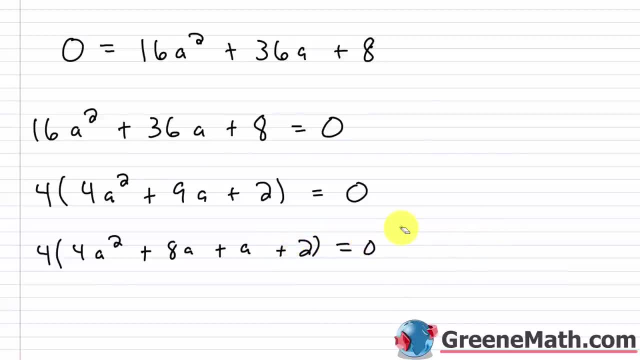 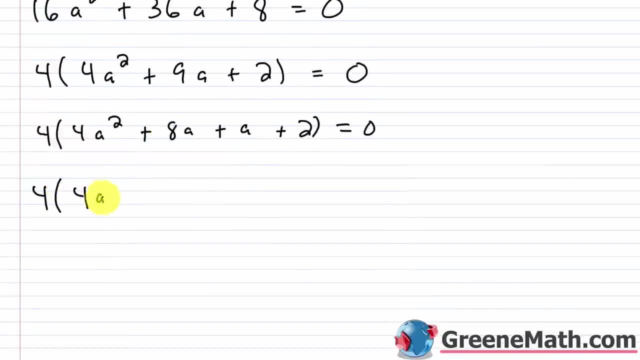 Okay, so let's erase this, and let's get our little room going. So I'd write 4, and the first group I could pull out of 4a, who would that leave me with? a plus 2. 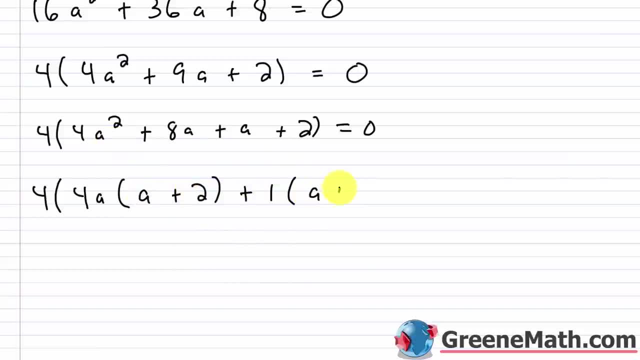 And the second group I'd just pull out of 1, and that would leave me with a plus 2. 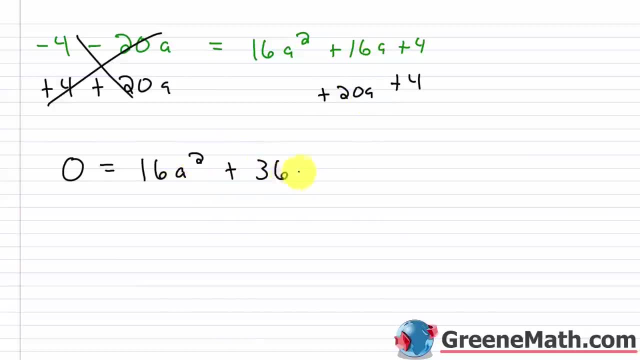 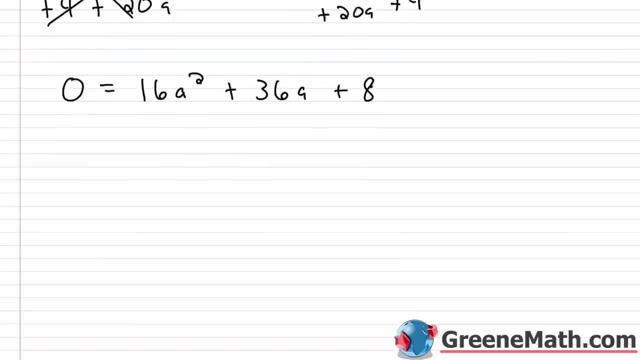 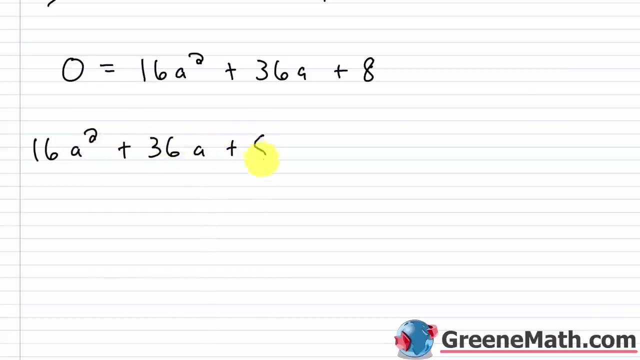 16a plus 20a is 36a, So plus 36a And then plus 8.. And again, I like the 0 on the right side. It doesn't matter, It's just personal preference. So I'm going to rewrite this as: 16a squared plus 36a plus 8 equals 0.. 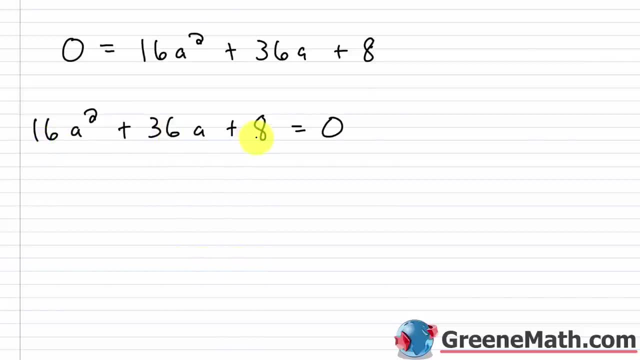 So before I move forward, I notice that I can pull a 4 out of everything. So if I pull a 4 out, this would be 4a squared Plus 9a plus 2. And this is equal to 0.. 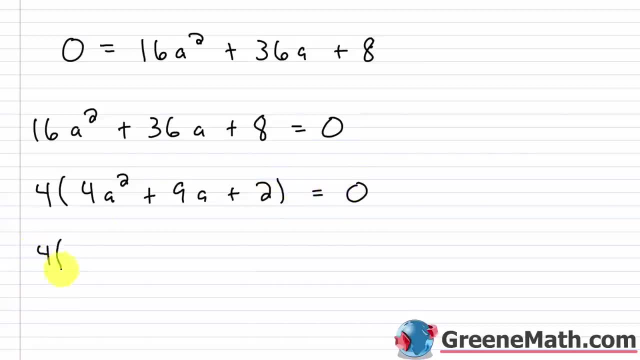 So to factor the inside here I'm going to use factoring by grouping. So give me two integers: whose product, whose product is 8 and whose sum is 9.. That's easy, That's 8 and 1.. So let's rewrite that middle term. 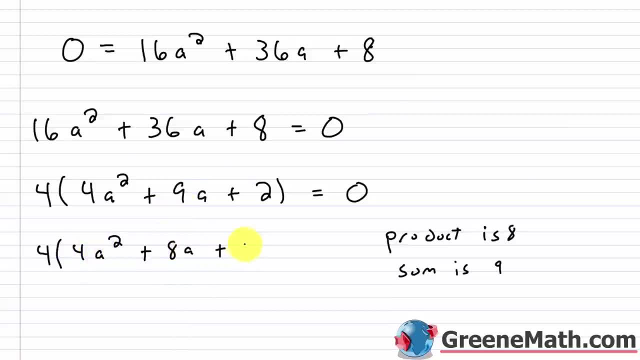 We'll have 4a squared plus 8a, plus a plus 2.. This is equal to 0.. So let's erase this And let's get our little room going. So I'd write 4.. In the first group I could pull out a 4a. 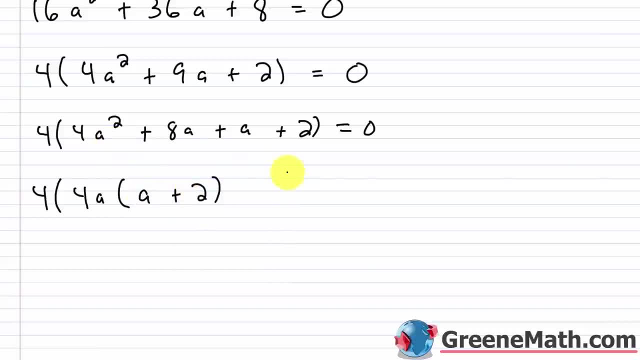 Who would that leave me with a plus 2.. In the second group, I just pull out a 1., And that would leave me with a plus 2.. Okay, So then this equals 0. And so what I'm going to do now? I'm going to factor out the common binomial factor. 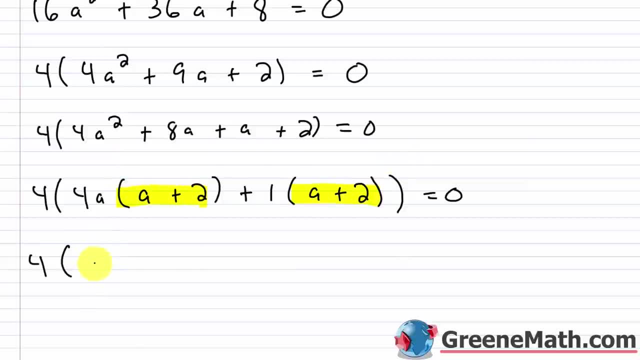 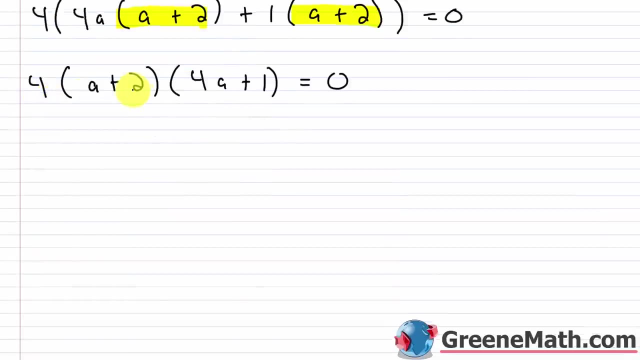 And that's this a plus 2 here. So if I pull that out I'd have a plus 2, that quantity times I'd have 4a plus 1.. Okay, this equals 0.. So now, in factored form, I have 4 times the quantity a plus 2 times the quantity 4a plus 1.. 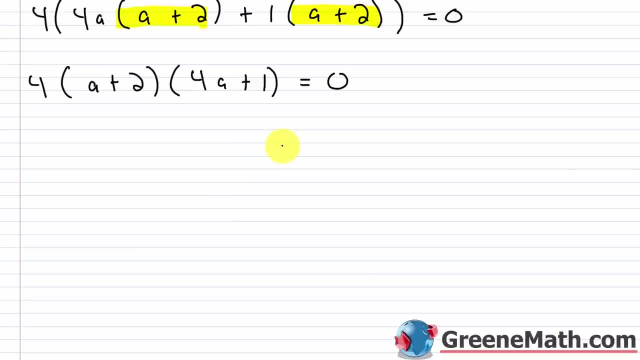 Okay, and then this equals 0. So, using my 0 product property, I set each factor with a variable equal to 0. So I don't need to set 4 equal to 0. That doesn't make any sense. I'd set a plus 2 equal to 0. 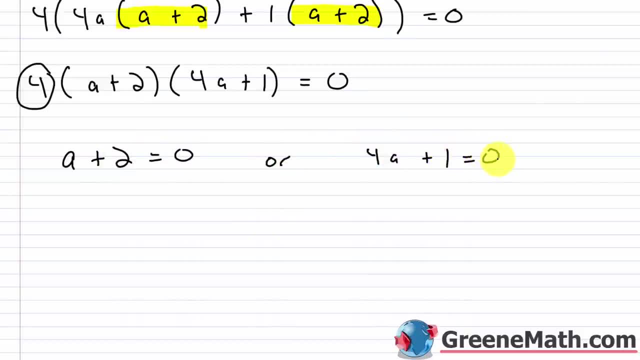 And I'd also set 4a plus 1 equal to 0.. So this is easy: Subtract 2 from each side, you get a equals negative 2.. For this one, I subtract 1 away from each side, I get 4a- equals negative 1.. Okay, so then this equals 0. 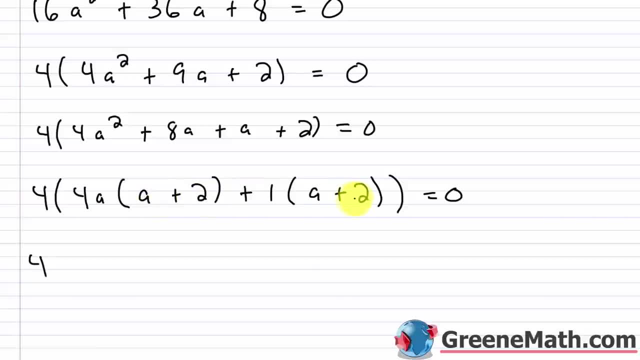 And so what I'm going to do now, I'm going to factor out the common binomial factor, and that's this a plus 2 here. So if I pull that out, I'd have a plus 2, that quantity, times, I'd have 4a plus 1. Okay, this equals 0. So now, in factored form, I have 4a plus 1. Okay, this equals 0. 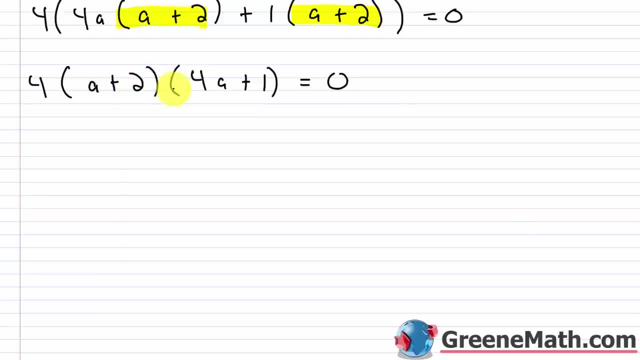 So in factored form, I have 4 times the quantity a plus 2 times the quantity 4a plus 1. Okay, and then this equals 0. So using my zero product property, I set each factor with a variable equal to 0. So I don't need to set 4 equal to 0, that doesn't make any sense. I'd set a plus 2 equal to 0, and I'd also set 4a plus 1 equal to 0. So this is easy. Subtract 2 from each side, you get a equals negative 2. 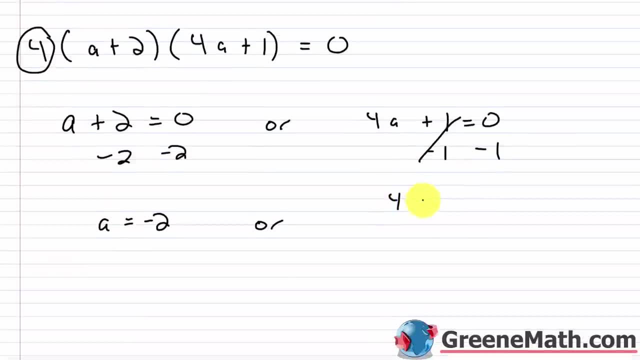 For this one, I subtract 1 away from each side, I get 4a equals negative 1. 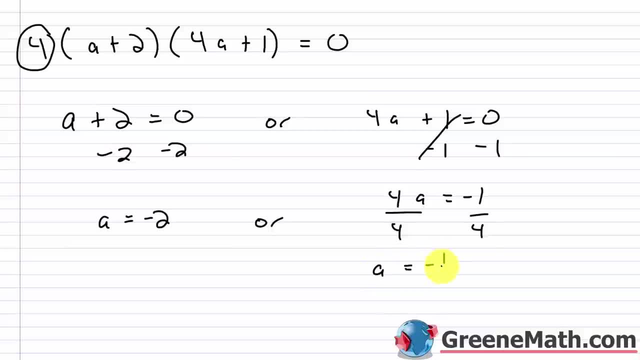 I divide both sides by 4, and I get a equals negative 1 fourth. 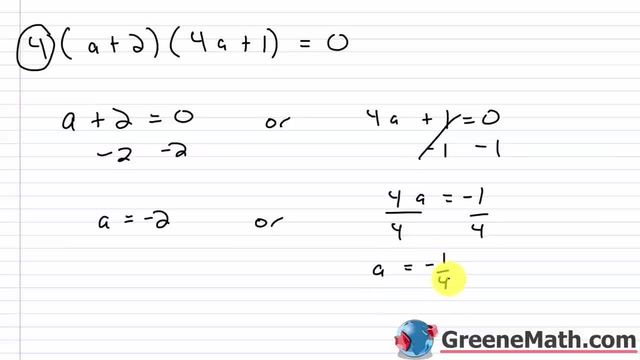 So a equals negative 2, or a equals negative 1 fourth. 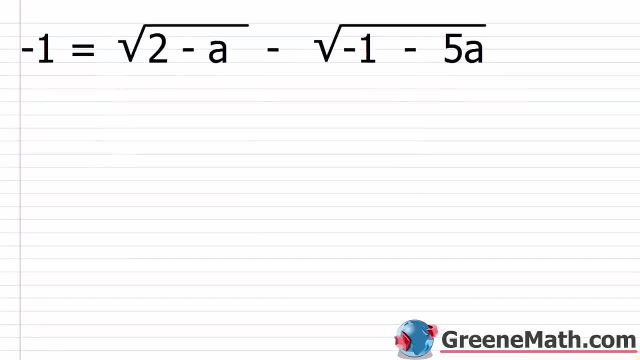 Now let's go back and let's check each one and make sure that they work in the original equation. 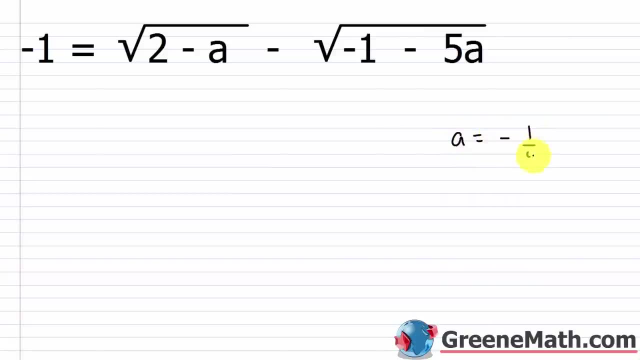 So we have a equals negative 1 fourth. And we have a is equal to negative 1 fourth. And we have a equals negative 1 fourth. And we have a is equal to negative 1 fourth. 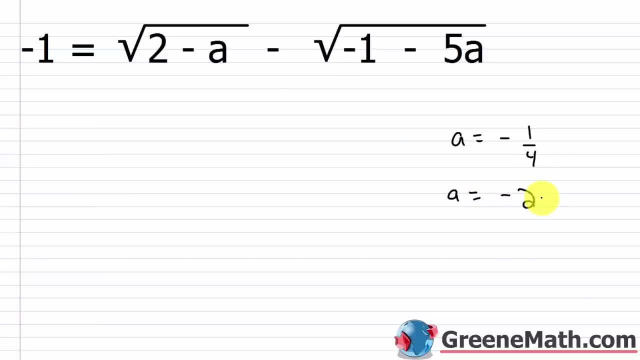 And we have a is equal to negative 2. So let's start out with a equals negative 2. 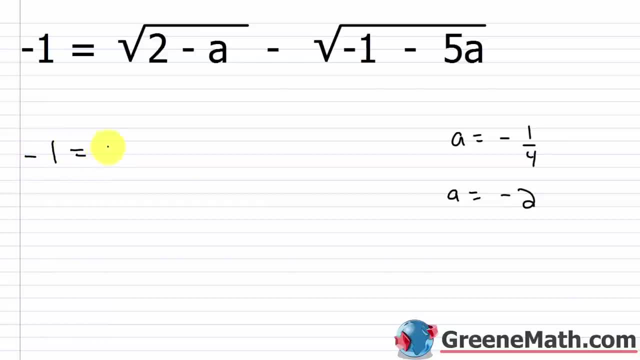 So if I plug that in, let's have negative 1 is equal to the square root of 2 minus a negative 2 is like 2 plus 2. So the square root of 4. And we might as well replace that with 2, we know what that is. So we'll have a 2 there minus the square root of negative 1 minus 5 times negative 2 is negative 10. So I'd have minus a negative 10, which is plus 10. Okay. 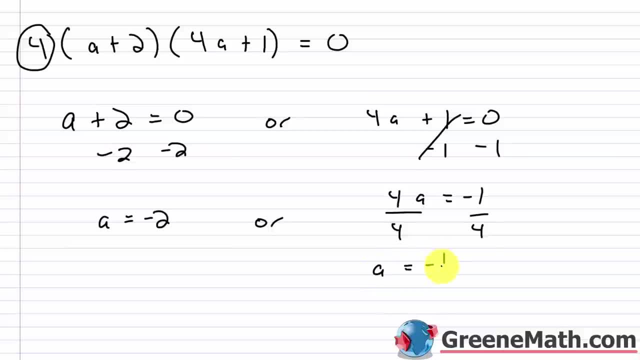 I divide both sides by 4, and I get a equals negative 1 fourth. So a equals negative 2, or a equals negative 1 fourth. Now Let's go back and let's check each one and make sure that they work in the original equation. 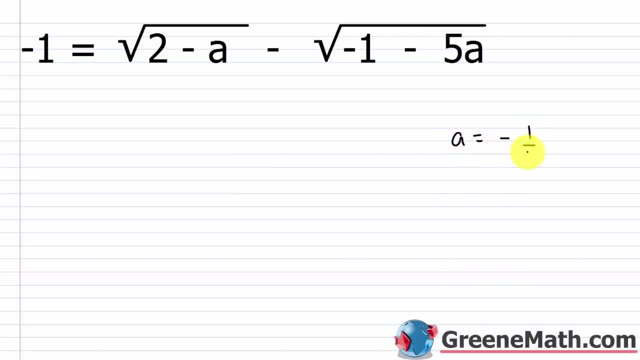 So we have a equals negative 1. fourth, and we have a is equal to negative 2.. So let's start out with a equals negative 2.. So if I plug that in, let's have: negative. 1 is equal to the square root of 2 minus a negative. 2 is like 2 plus 2.. 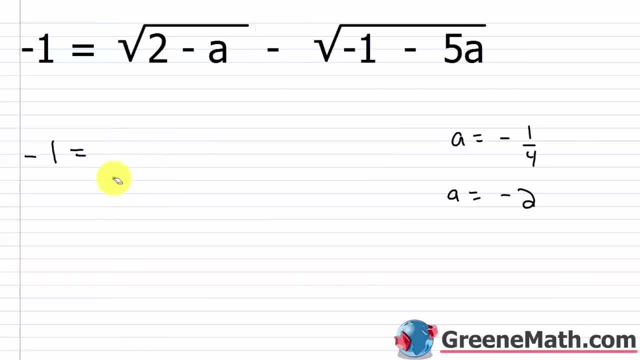 So the square root of 4.. We might as well replace that with 2.. We know what that is, So We'll have a 2 there, Minus the square root of negative 1. minus 5 times negative 2 is negative 10.. 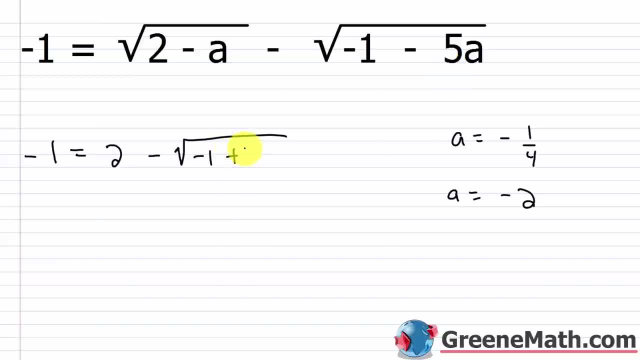 So I'd have minus a negative 10, which is plus 10.. So really this would be 9.. We know the square root of 9 is 3.. 2 minus 3 is negative 1. So that one works out just fine. 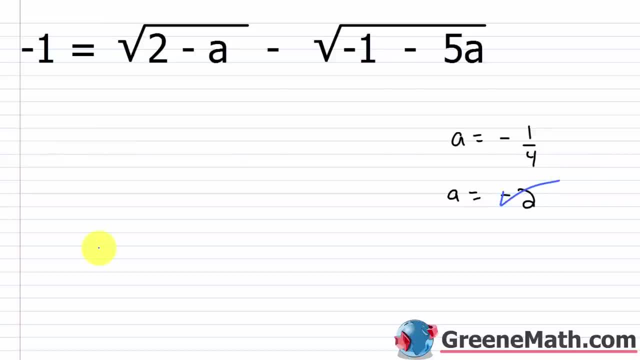 So this is a solution for our equation. So let's take a look at a equals negative 1 fourth now. So we have: negative 1 is equal to the square root of 2.. We have minus a negative 1 fourth. That's like 2 plus 1 fourth. 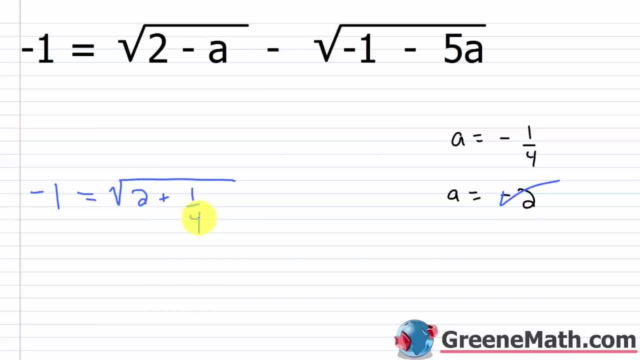 Okay, So 2 plus 1 fourth. Now, to deal with the fact that we have fractions involved, I could write 2 as 8 fourths, Right, 8 fourths, And really I could write this as 9 fourths. 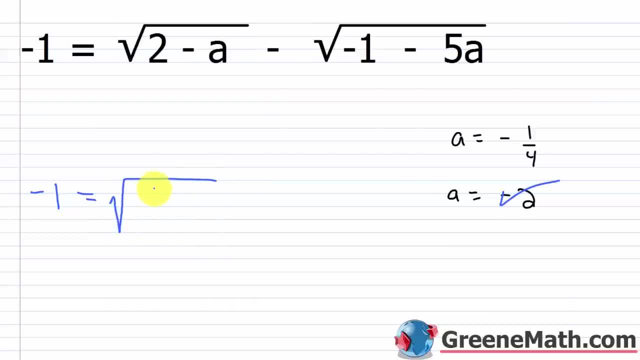 So the square root, the square root of 9, fourths, And we know we can write that as the square root of 9 over the square root of 4.. The square root of 9 is 3.. The square root of 4 is 2.. 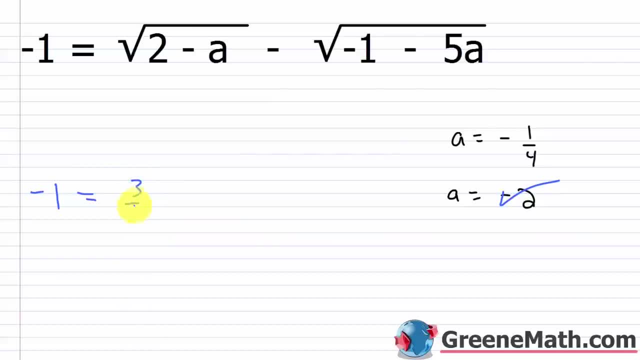 So this is really 3 halves. This is 3 halves, Then minus Over. here I have the square root of negative 1 minus 5 times a negative 1 fourth. So negative times negative is positive. So this would be positive 5 fourths. 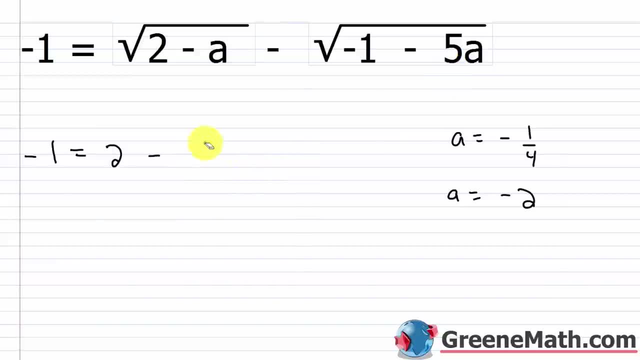 So really, this would be 9. We know the square root of 9 is 3. 2 minus 3 is negative 1. So that one works out just fine. 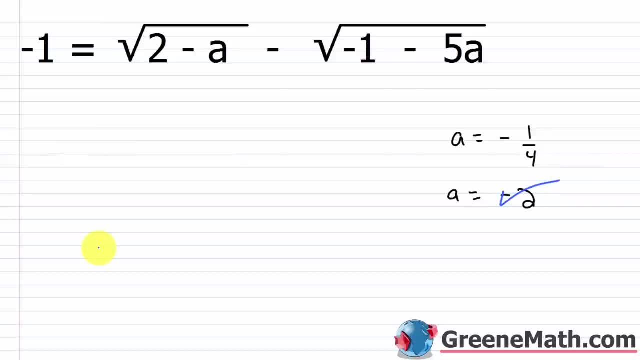 So this is a solution for our equation. So let's take a look at a equals negative 1 fourth now. 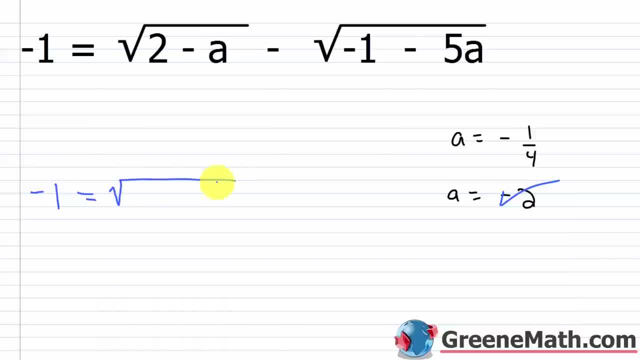 So we have negative 1 is equal to the square root of 2. 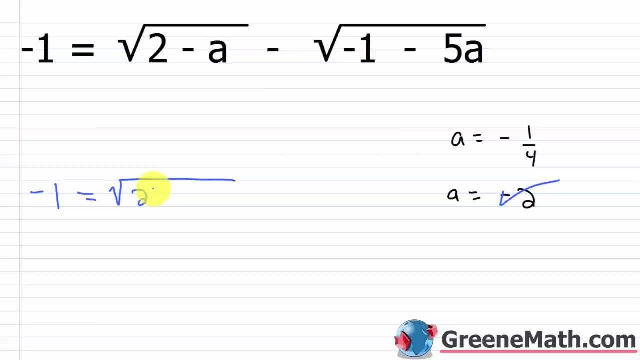 We have minus a negative 1 fourth, that's like 2 plus 1 fourth, okay? So 2 plus 1 fourth. Okay. 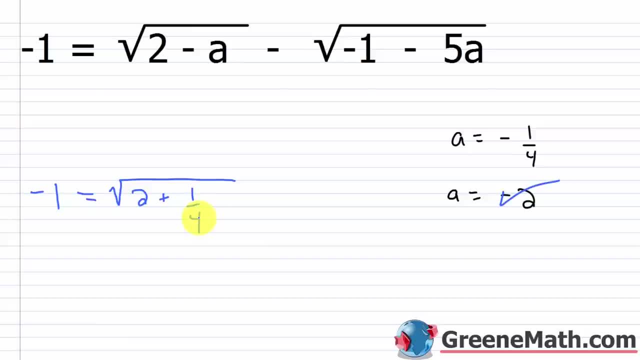 Now, to deal with the fact that we have fractions involved, I could write 2 as 8 fourths, right? 8 fourths. And really, I could write this as 9 fourths. So the square root, the square root of 9 fourths. And we know we can write that as the square root of 9 over the square root of 4, square root of 9 is 3, square root of 4 is 2. So this is really 3 halves. This is 3 halves. 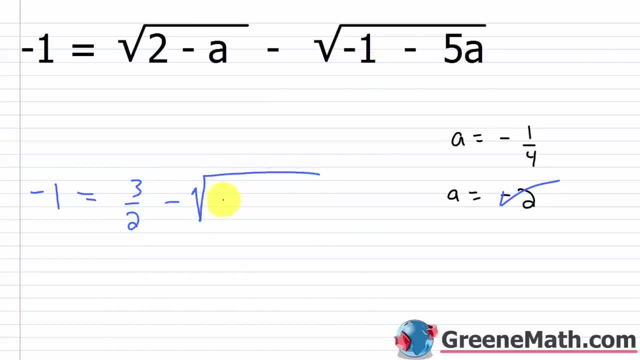 Then minus. Over here, I have the square root. Of negative 1 minus 5 times a negative 1 fourth. So negative times negative is positive, so this would be positive 5 fourths. So plus 5 fourths. And of course, to get a common denominator here, I would simply write this as negative 4 over 4. 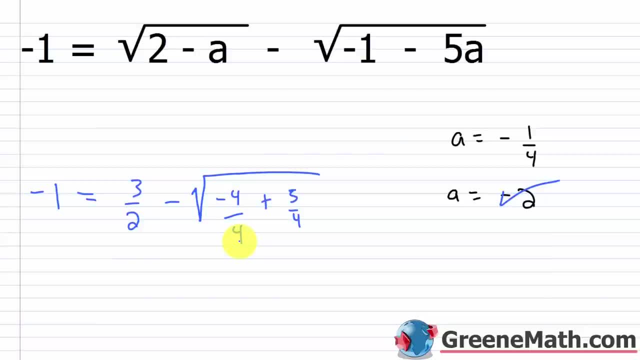 Negative 4 over 4. Negative 4 plus 5 is 1. So this would be 1 fourth. This would be 1 fourth. And again, I can break this down into the square root. Square root of 1 over the square root of 4. Square root of 1 is 1. Square root of 4 is 2. So this is 1 half. 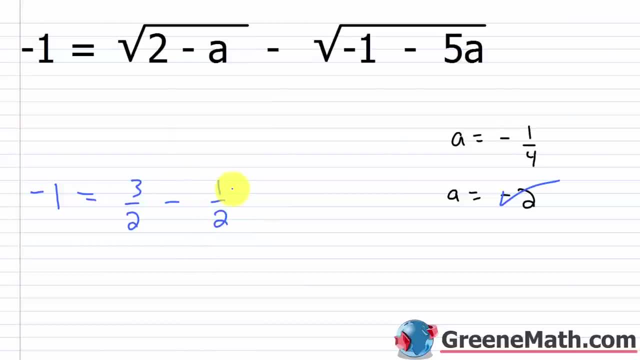 This is 1 half. So 3 minus 1 is 2. And this would be over 2. 2 over 2 is equal to 1. 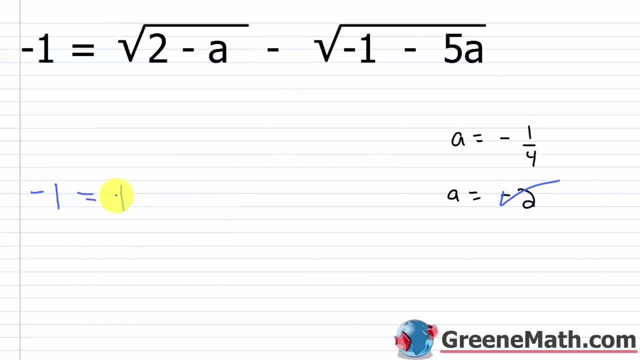 So what do I get here? I get that negative 1 is equal to 1. That's not right. Negative 1 doesn't equal 1. And this is part of the problem again. 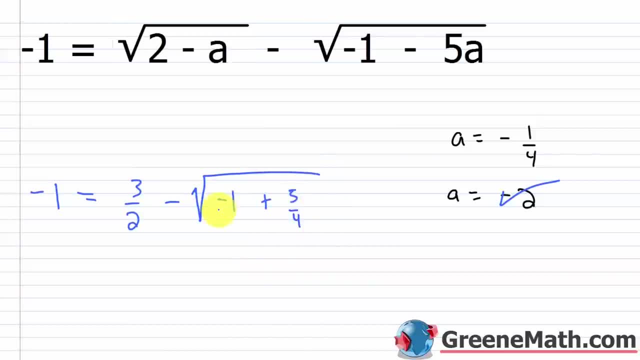 So plus 5. fourths, And of course, to get a common denominator here, I would simply write this as negative 1. fourth, I would simply write this as negative 4 over 4.. Negative 4 over 4. Negative 4 plus 5 is 1.. 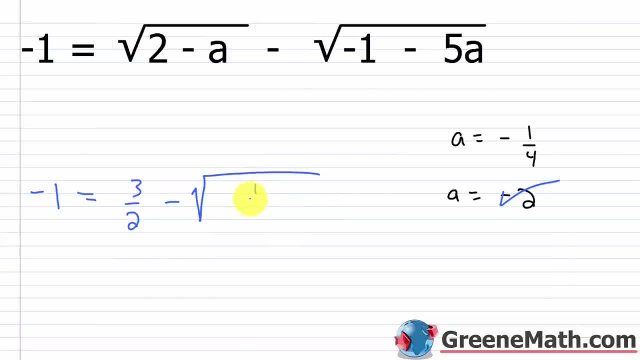 So this would be 1 fourth. This would be 1 fourth, And again I can break this down into the square root of 1 over the square root of 4.. The square root of 1 is 1.. The square root of 4 is 2.. 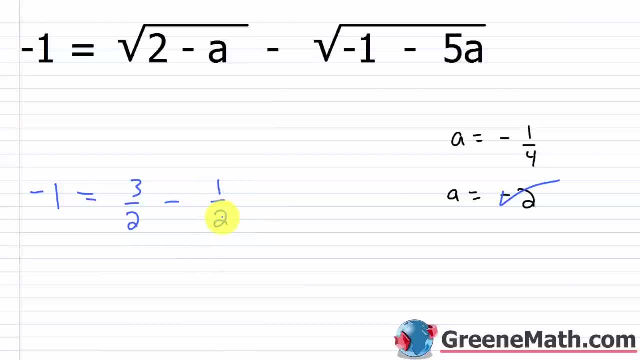 So this is 1 half, This is 1 half. So 3 minus 1 is 2.. And this would be over 2.. 2 over 2 is equal to 1.. So what do I get here? I get that negative 1 is equal to 1.. 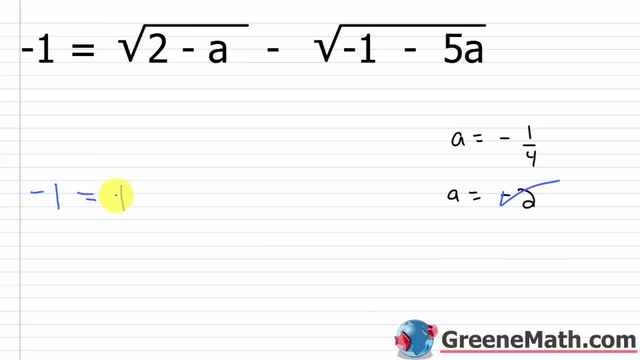 That's not right. Negative 1 doesn't equal 1.. And this is part of the problem again. When you use that squaring property of equality, you're going to end up with solutions that don't work in the original equation. So this one does not work. 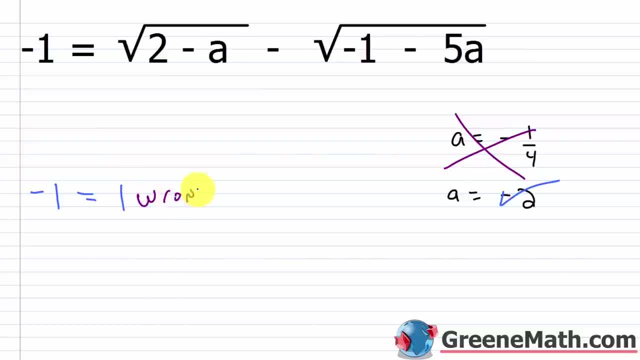 It's not a valid solution in the original equation. This is wrong, Not a true statement, And so the solution here is a equals negative 2.. And that's your answer. That's your only solution. Hello and welcome to Algebra 1, Lesson 59.. 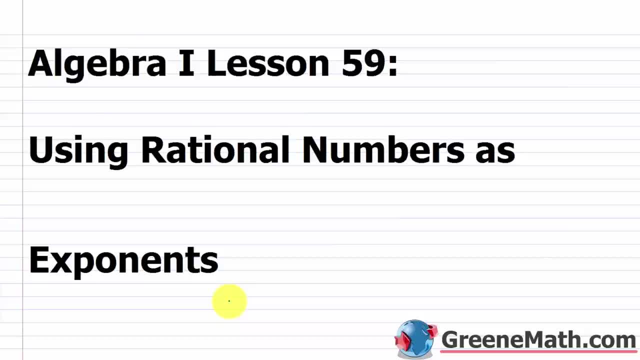 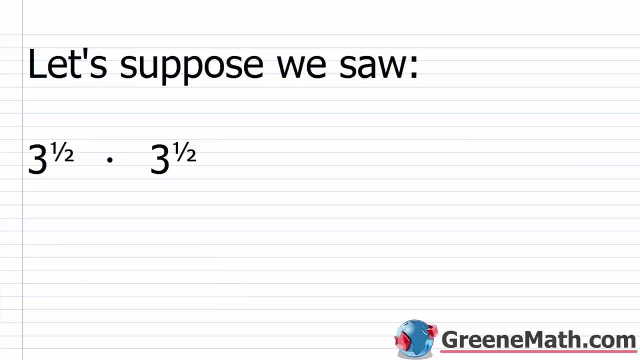 In this video, we're going to learn about using rational numbers as exponents, which is also known as working with fractional exponents. Alright, so we're going to kind of just jump right in. This is not a very hard topic to wrap your head around. 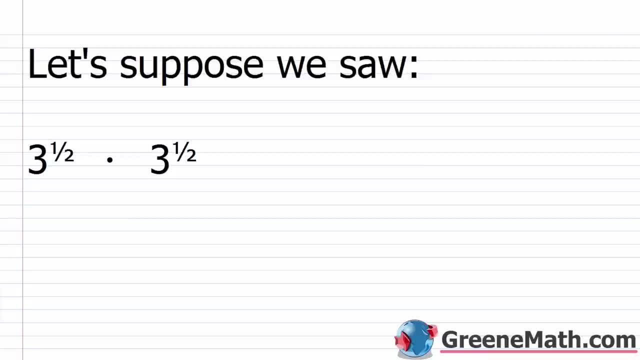 And it's something that is going to dramatically increase your speed when you're simplifying radicals moving forward. So let's suppose we saw something like 3 to the power of 1 half times 3 to the power of 1 half. So at this point we have all the tools that we need. 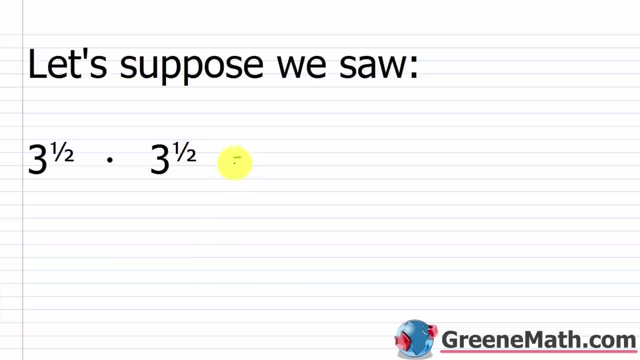 to simplify something like this: Now we know that from the rules of exponents, we would keep our base 3 the same, So that stays the same, And then we would add the exponents. We would add the exponents because we're multiplying. 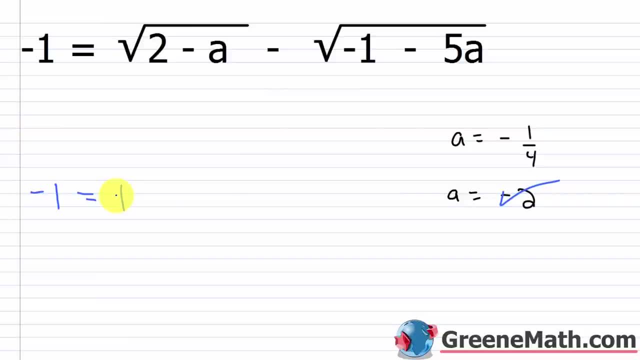 When you use that squaring property of equality, you're going to end up with solutions that don't work in the original equation. So this one does not work. It's not a valid solution in the original equation. This is wrong. Not a true statement. 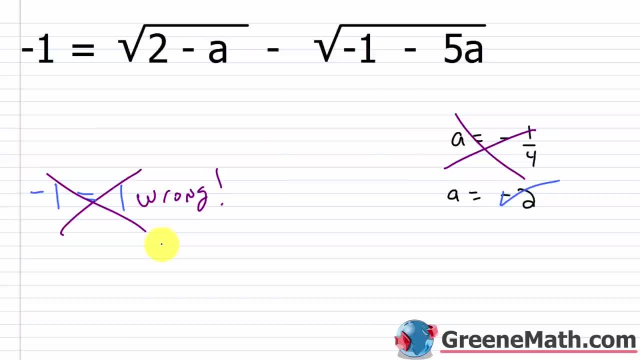 And so the solution here is a equals negative 2. And that's your only solution. 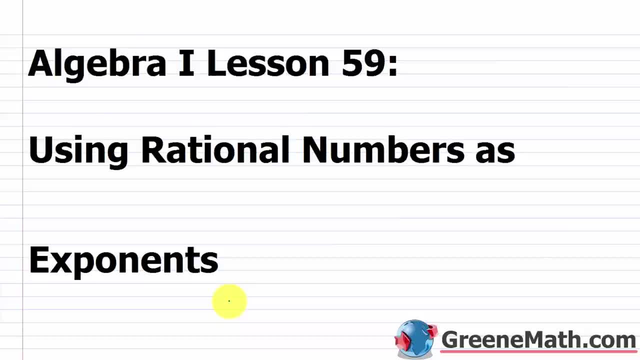 Hello and welcome to Algebra 1 Lesson 59. 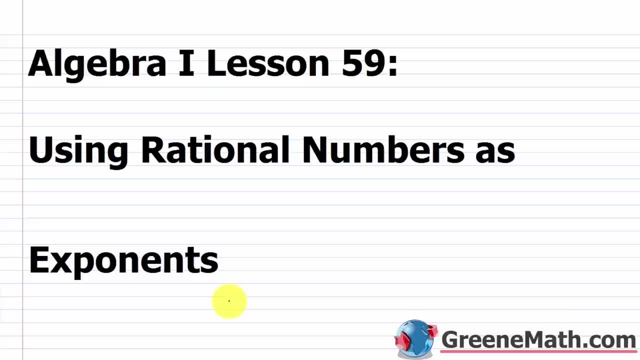 In this video, we're going to learn about using rational numbers as exponents, which is also known as working with fractional exponents. 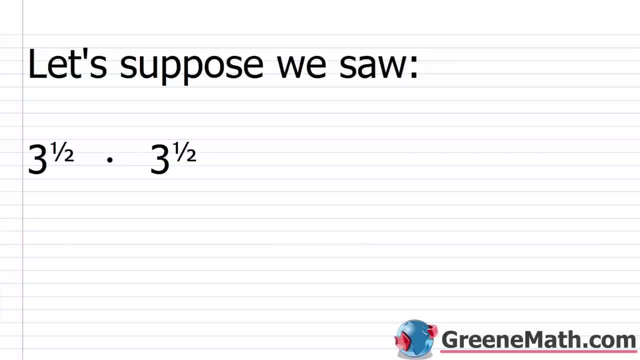 All right, so we're going to kind of just jump right in. This is not a very hard topic to wrap your head around. 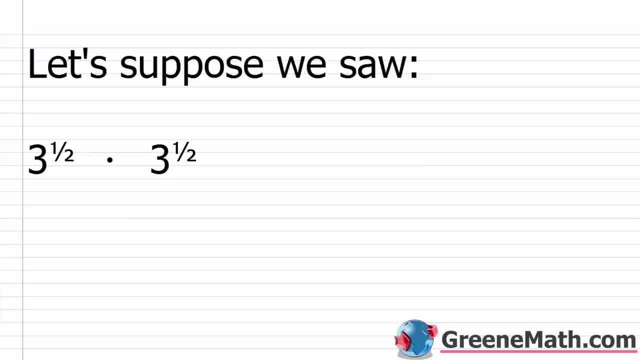 And it's something that is going to dramatically increase your speed when you're simplifying radicals moving forward. 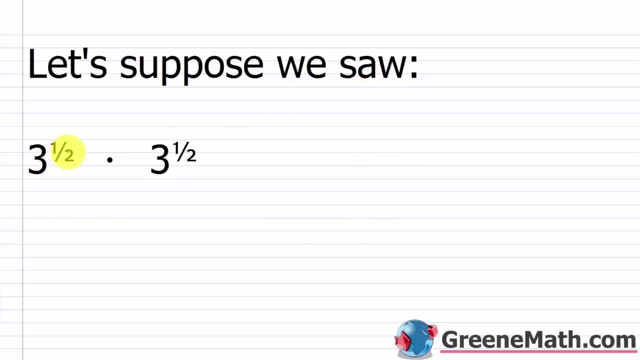 So let's suppose we saw something like 3 to the power of 1 half times 3 to the power of 1 half. So at this point, we have all the tools that we need to simplify something like this. Now. 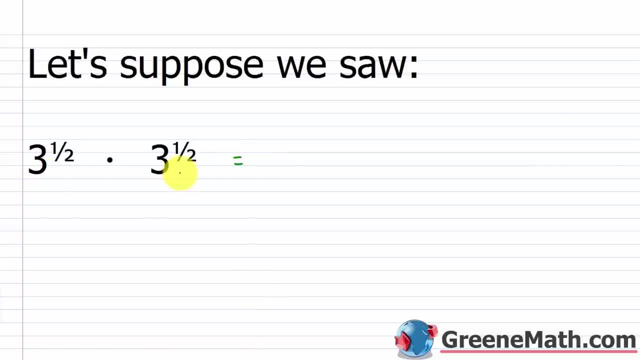 Let's say that from the rules of exponents, we would keep our base 3 the same. That stays the same. And then we would add the exponents. We would add the exponents because we're multiplying. So this would be 3 to the power of 1 half plus 1 half. Now we already have a common denominator, so this is pretty easy to do. This would be 3 to the power of 1 plus 1 is 2 over the common denominator of 2. And then 2 over 2 is just 1. So this would be 3. 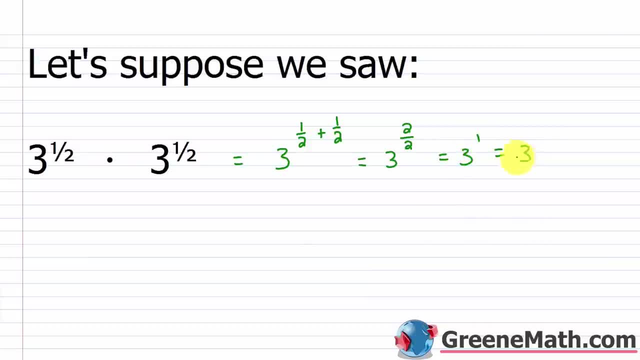 3 to the power of 1 which is just 3. 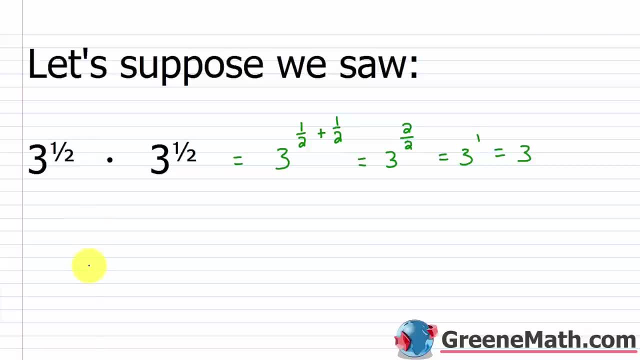 Now having seen me do this example, what can you guess is going to be another way that we can write 3 to the power of 1 half? 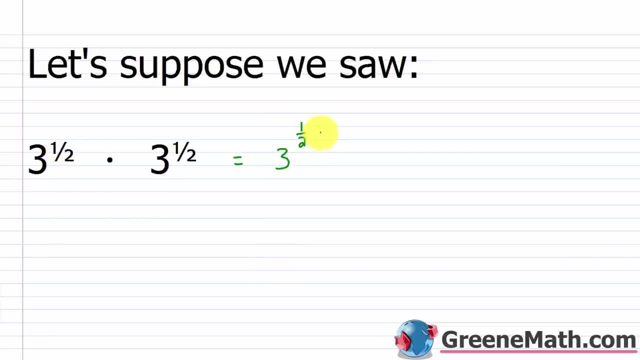 So this would be 3 to the power of 1 half plus 1 half. Now we already have a common denominator, So this is pretty easy to do. This would be 3 to the power of 1 plus 1 is 2. 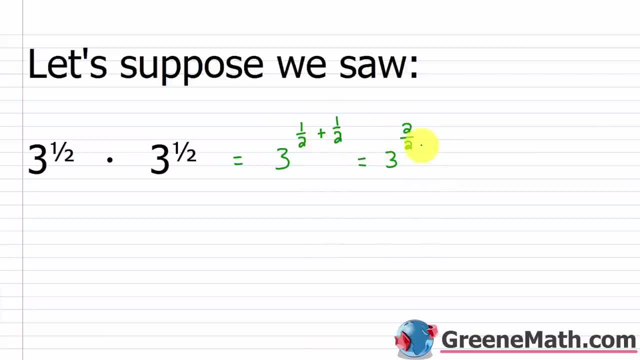 over the common denominator of 2.. And then 2 over 2 is just 1.. So this would be 3 to the power of 1, which is just 3.. Now, having seen me do this example, what can you guess? 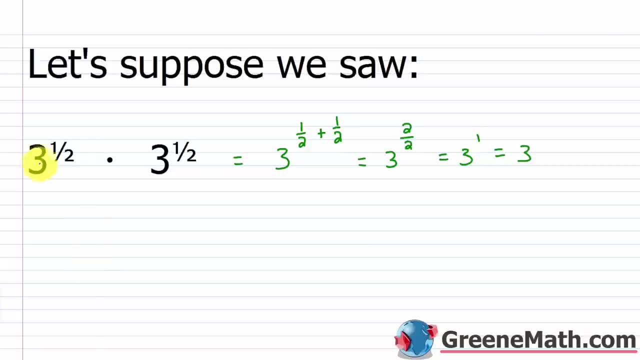 is going to be another way that we can write 3 to the power of 1 half. Well, it's going to be the square root of 3, right, Because the square root of 3 times the square root of 3 is going to equal what? 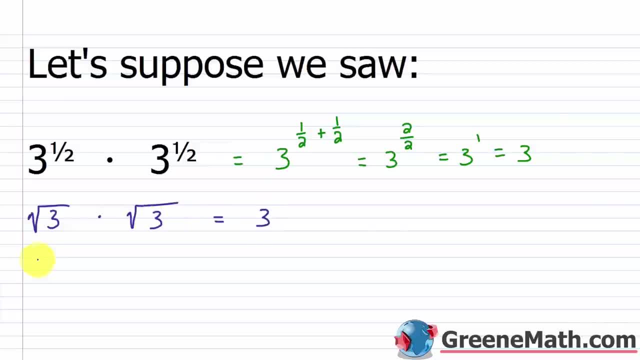 At the end of the day, it's going to equal 3.. Square root of 3 times square root of 3 is 3.. Square root of 2 times square root of 2 is 2.. Square root of, let's say, 4. 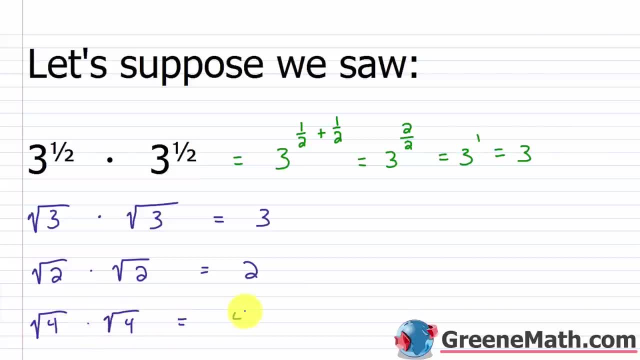 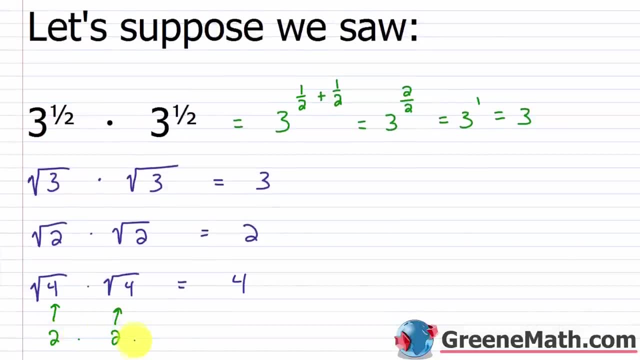 times square root of 4 is what It's, 4.. And we know this one because square root of 4 is a rational number. This would be 2 times 2,, which we know is 4, right, So we can prove the rule by looking at that. 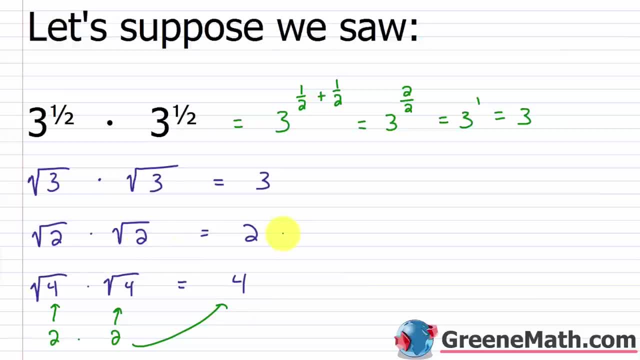 So in each case I could rewrite these. I could say: this is really 2 to the power of 1 half times 2 to the power of 1 half, which equals 2, right, It's 2 to the power of 1 half plus 1 half. 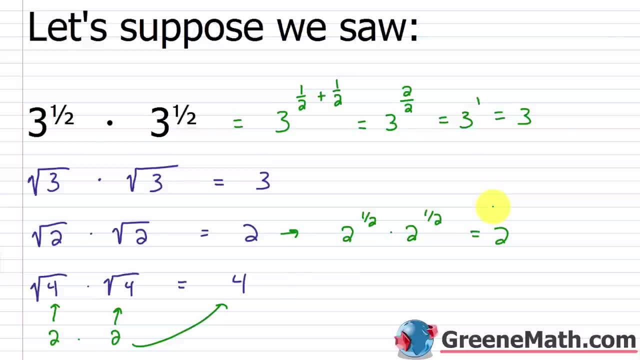 which is 2 to the power of 1.. In this case, I can say: this is what: 4 to the power of 1 half times 4 to the power of 1 half, which is 4.. So having a number raised to the power of 1 half, 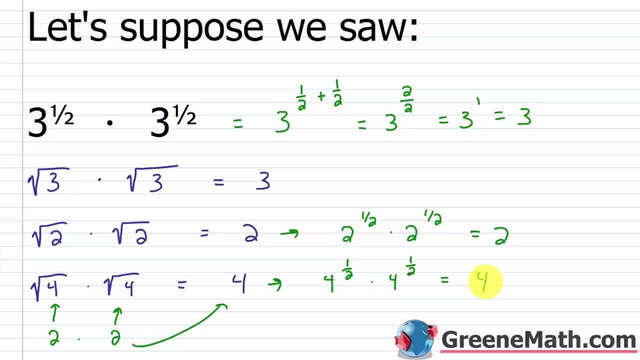 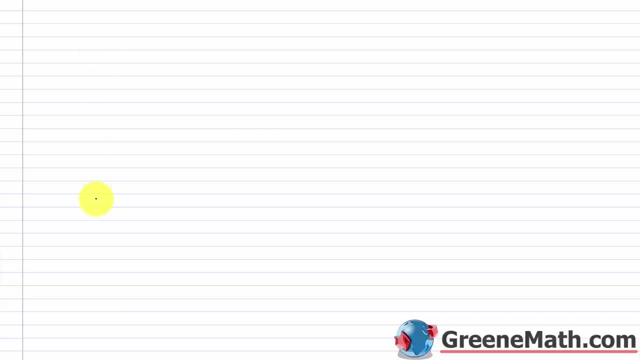 is the same thing as taking the square root of the number. It's just how we write it with exponents. Now, as something that's a little bit more complicated, let's say we stay with the number 3.. And we saw 3 raised to. 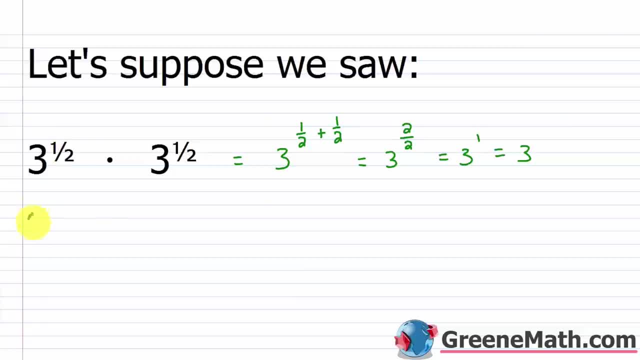 Well it's going to be the square root of 3, right? Because the square root of 3 times the square root of 3 is going to equal what? At the end of the day, it's going to equal 3. Square root of 3 times square root of 3 is 3. 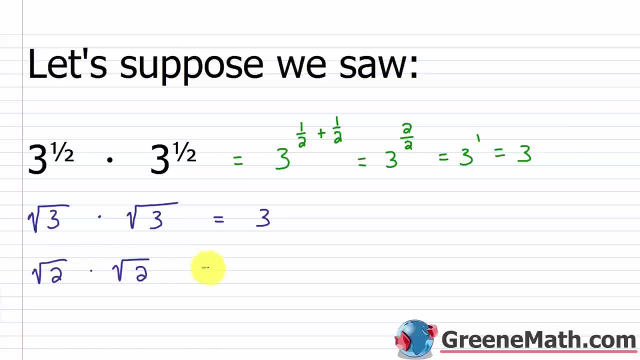 Square root of 2 times square root of 2 is 2. 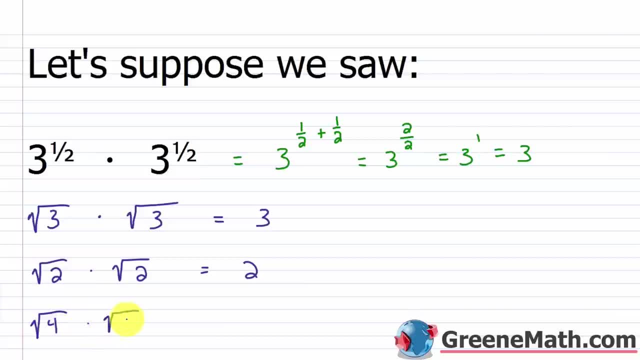 Square root of, let's say, 4 times square root of 4 is what? It's 4. 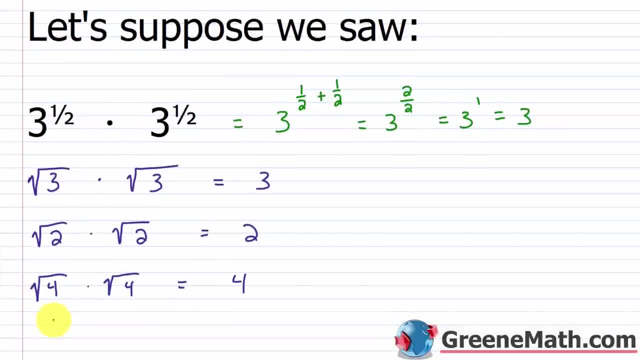 And we know this one because the square root of 4 is a rational number. This would be 2 times 2, which we know is 4, right? 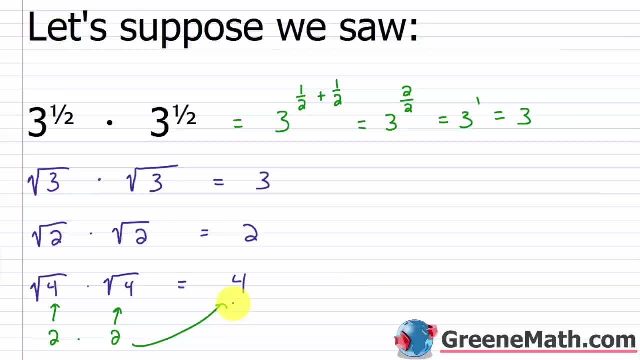 So we can prove the rule by looking at that. So in each case, I could rewrite these. I could say this is really 2 to the power of 1 half. I could say this is really 2 to the power of 1 half. I could say this is really 2 to the power of 1 half. 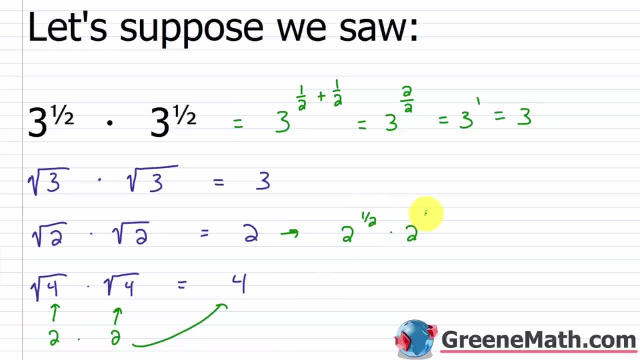 So it's 2 to the power of 1 half times 2 to the power of 1 half, which equals 2. Right? 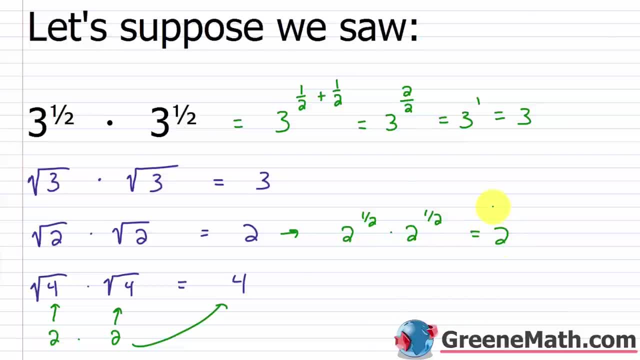 It's 2 to the power of 1 half plus 1 half, which is 2 to the power of 1. In this case, I can say this is what? 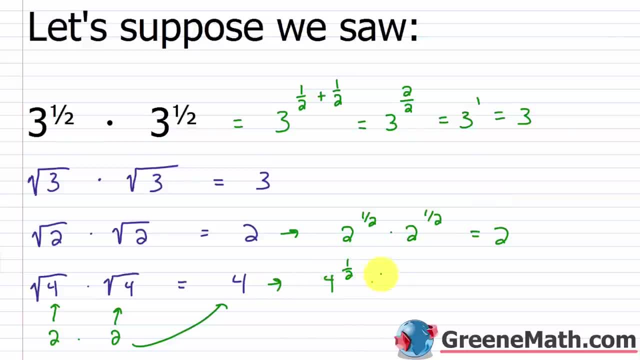 It's 4 to the power of 1 half times 4 to the power of 1 half, which is 4. 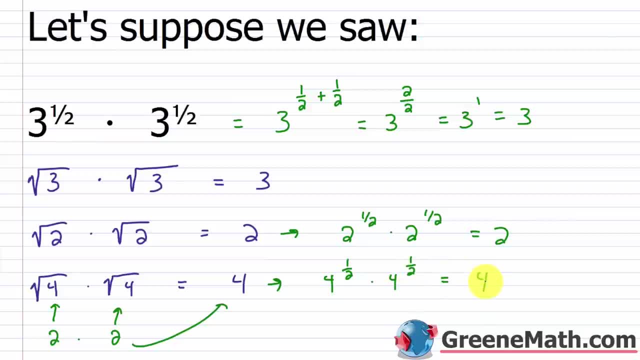 So having a number raised to the power of 1 half is the same thing as taking the square root of the numbers. Just how we write it. 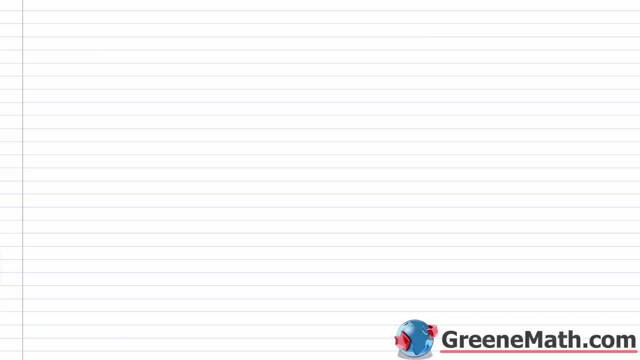 with exponents. Now as something that's a little bit more complicated, let's say we stay with the number three. And we saw three raised to, I don't know, let's say the one third power, okay, the power of one third. So then I would multiply this by three to the power of one third again, and then one more time. So again, using our rules for exponents, what would this be equal to? Well, I 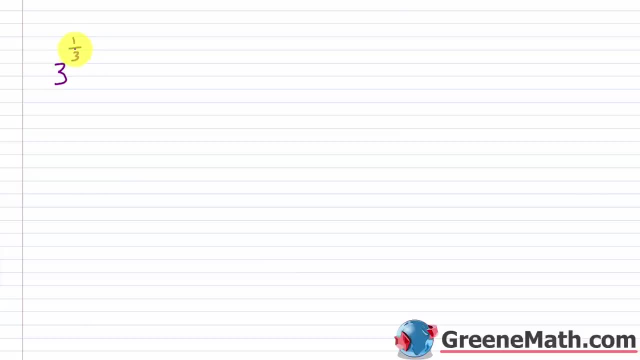 I don't know. let's say the 1 third power. Okay, the power of 1 third. So then I would multiply this by 3 to the power of 1 third again, and then one more time, So again using our rules for exponents. 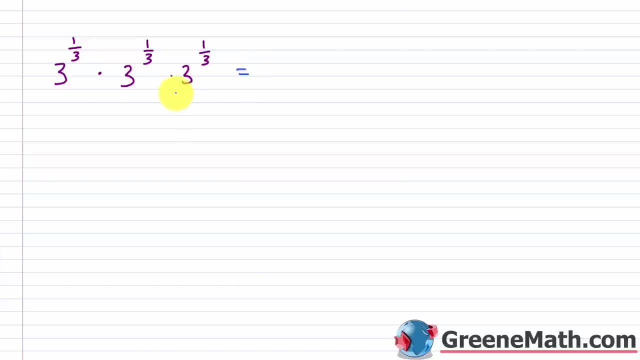 what would this be equal to? Well, I have the same base, so that stays the same, And then I would just add the exponents. So 1 third plus 1 third plus 1 third is equal to what It's equal to 1, right. 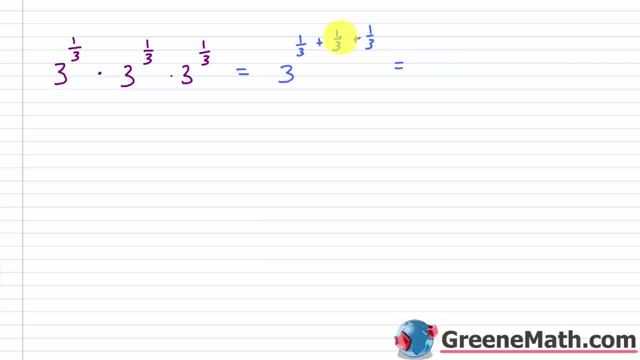 1 plus 1 plus 1 is 3.. 3 over that common denominator of 3 would be 1.. So this is 3 to the power of 3 thirds, which is equal to 3 to the power of 1 or just 3.. 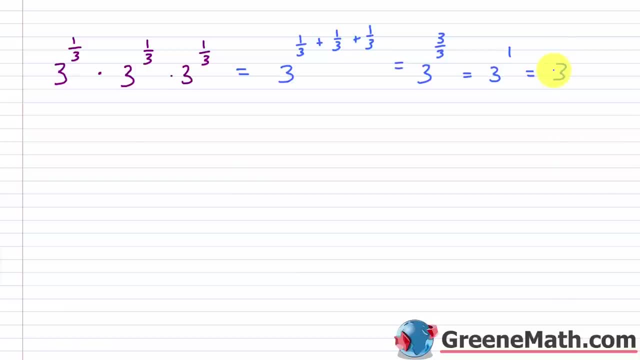 So, after having seen the last example, what would you guess is another way that we could write 3 to the power of 1, third, We could do the cube root of 3.. The cube root of 3.. Alright, because the cube root of 3 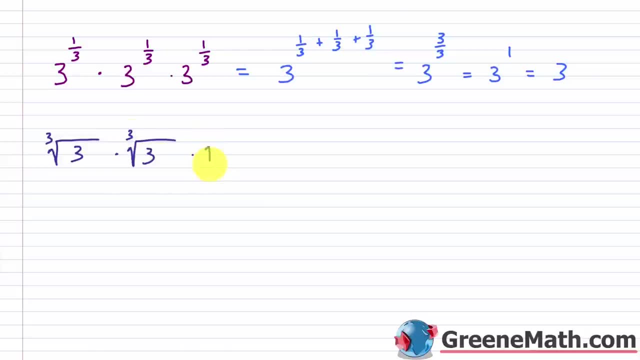 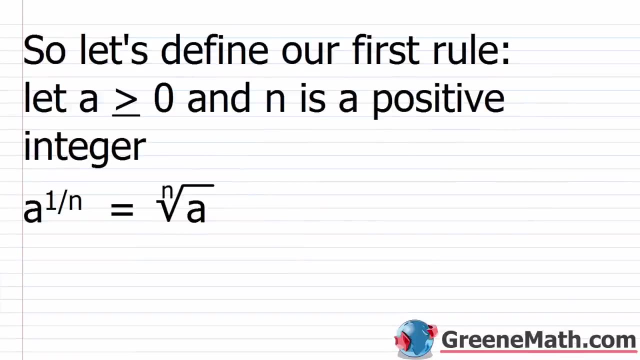 times the cube root of 3 times the cube root of 3 is equal to 3.. So now that we've seen a few examples, let's define our first rule. So we want to let a be greater than or equal to 0.. 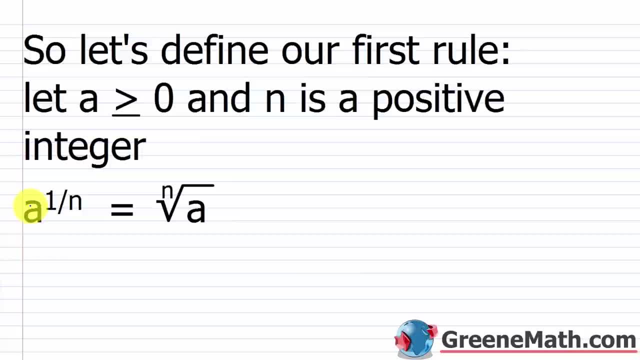 So this just means that a, which is right here, is going to be non-negative. And then we're also going to say that n is going to be positive. okay, It's going to be a positive integer. more specifically, Now, so that means that n can't be 0. 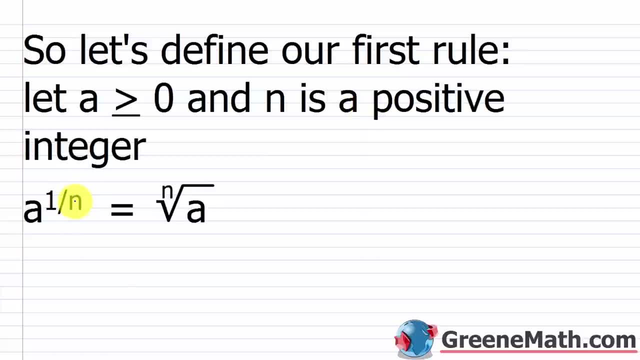 And n is in the denominator, so that's why it can't be 0. And also n is not going to be negative. okay, Now, when we have these conditions that are met, we can say that a raised to the power of 1 over n. 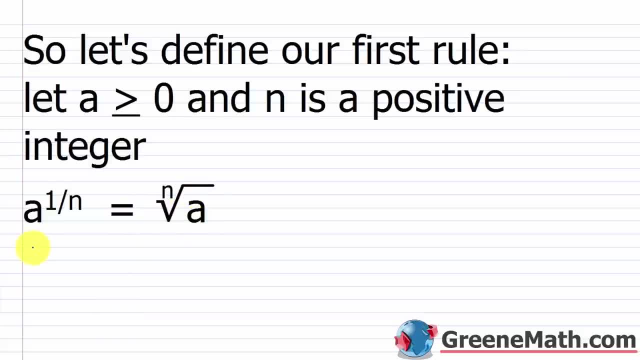 is equal to the nth root of a. So in other words, this, when we're looking at it in exponential form, is the base, And when we transform it over to this format, n is going to be the radicand. Then here, n is your denominator. 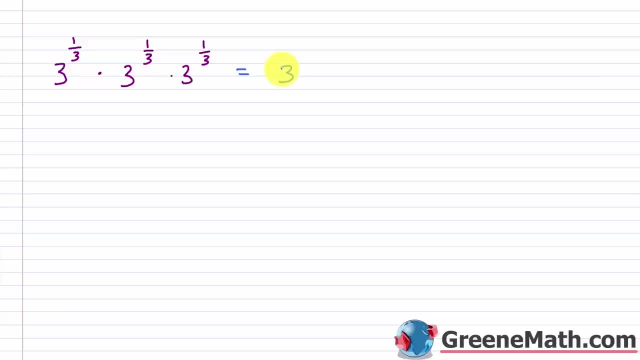 have the same base, so that stays the same. And then I would just add the exponents. So one third plus one third plus one third is equal to what? It's equal to one, right? One plus one plus one is three. Three over that common denominator of three would be one. So this is three to the power 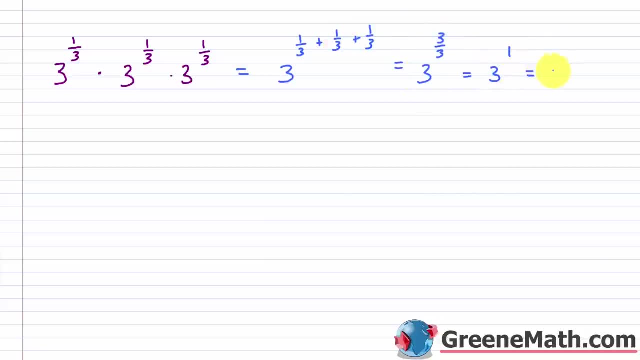 of three thirds, which is equal to three to the power of one, or just three. So after having seen the last example, what would you guess? 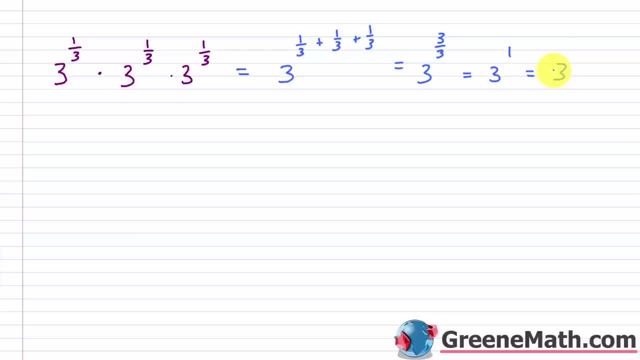 Is another way that we could write three to the power of one third. We could do the cube root of three, the cube root of three, right? Because the cube root of three times the cube root of three times the cube root of three is equal to three. So now that we've seen a few examples, let's define 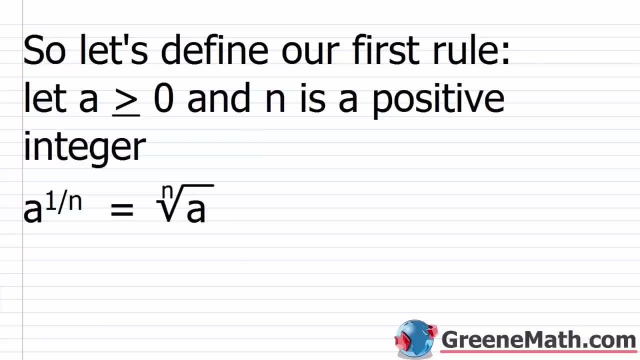 our first rule. So we want to let a be greater than or equal to zero. So this just means that a, which is right here, is going to be non-negative. And then we're also going to say that n is going to be positive. Okay, it's going to be a positive integer more specifically. Now, so that means that n can't be zero. And n is in the denominator, so that's why it can't be zero. And also n is not going to be negative. Okay. Now, when we have these conditions that are met, we can say that a raised to the 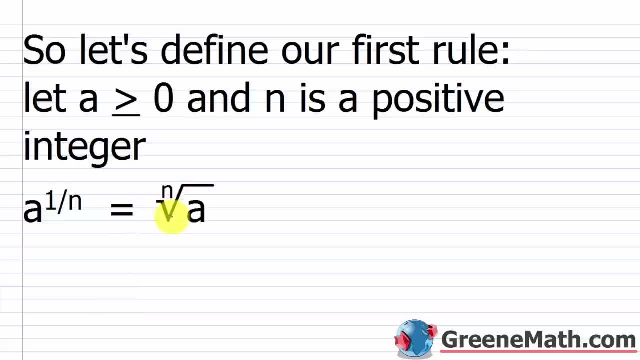 power of one over n is equal to the nth root of a. 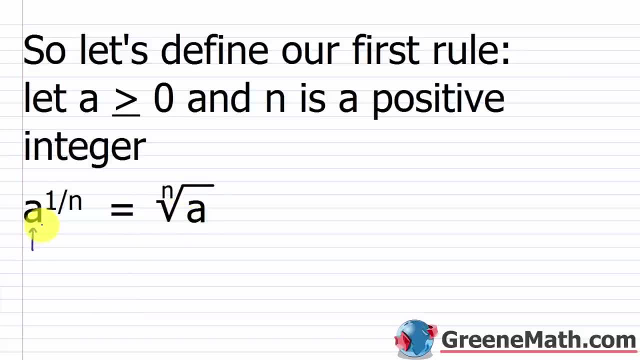 So in other words, this, or looking at it in exponential form, is the base. And when we transform it over to this format, it's going to be the radicand. Then here, n is your denominator. This is the denominator. 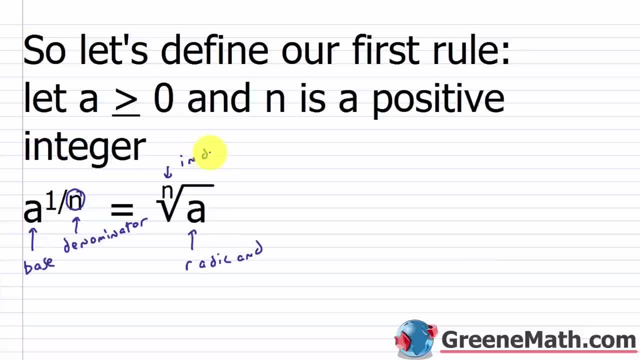 And when we move over here, it becomes the index. Now, I suggest that you write this particular thing down on a flash flash. Now, I suggest that you write this particular thing down on a flash flash. Now, I suggest that you write this particular thing down on a flash card. Okay. And what you want to do is, as we go through the examples here, keep your flash card out, pause the video. And then try to do it yourself. 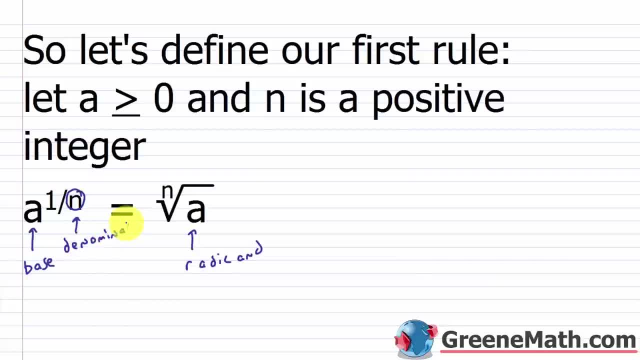 This is the denominator, And when we move over here it becomes the index. Now I suggest that you write this particular thing down on a flashcard, okay, And what you want to do is, as we go through the examples here, 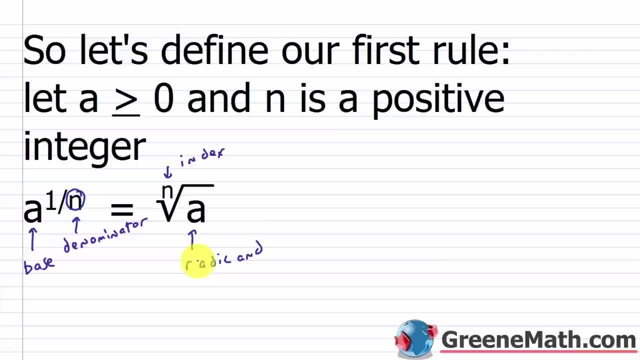 keep your flashcard out, pause the video and then try to do it yourself. okay, You can even do this when you're doing your practice problems or your homework. okay, After about 10 problems or so, you're going to memorize this generic formula. 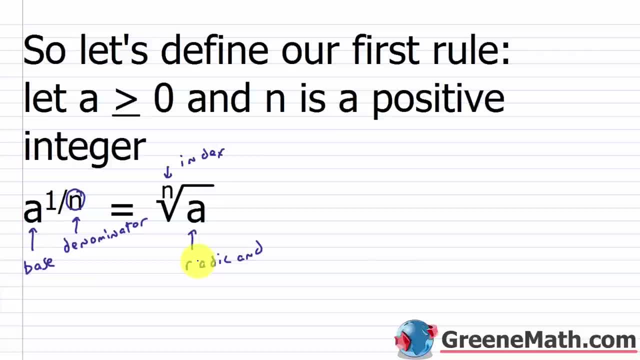 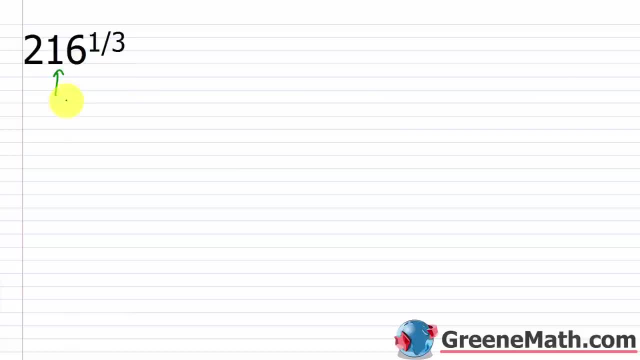 and you're going to do this without having to look at that flashcard. So let's start out with 216, raised to the power of 1 third. So we know that this is going to end up being our radicand. Okay, so let me write 216.. 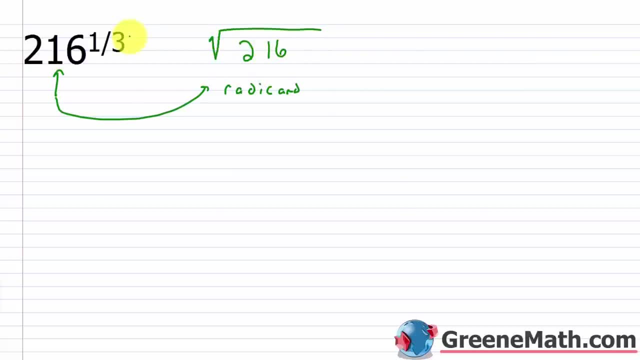 And let me write 216.. I'm going to write the radical, And we know that 3 is going to end up being the index. Okay, that's going to end up being the index. Okay, again, just straight from your flashcard. 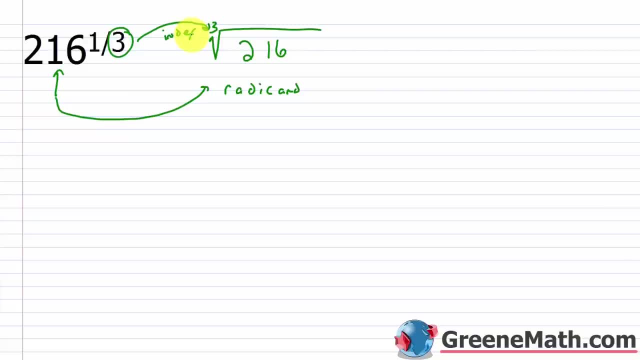 So we end up with the cube root of 216.. And most of you know at this point that that's going to be 6.. All right, that's going to be 6.. 6 times 6 is 36.. 36 times 6, once more, is 216.. 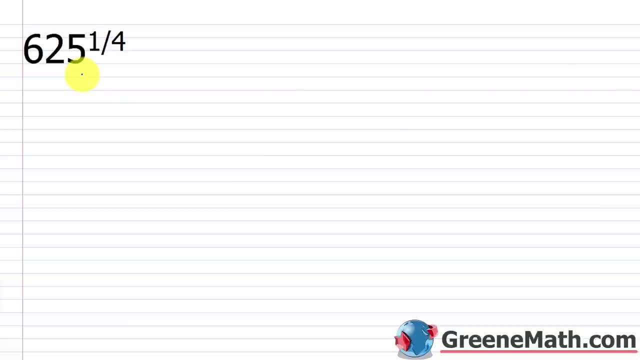 What about something like 625 to the 1 fourth power? So again, this part right here would be the radicand And it would be the fourth root right, Because this would be your index. So again, this would be the index. 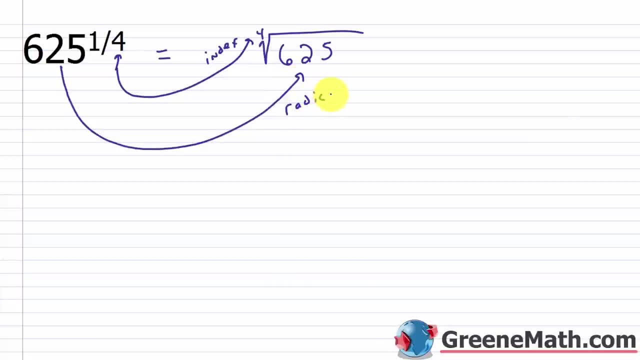 And then this would end up being the radicand. So I have the fourth root of 625.. And that's equal to 5, right? 5 times 5 is 25.. 25 times 5 is 125.. And then 125 times 5 is 625. 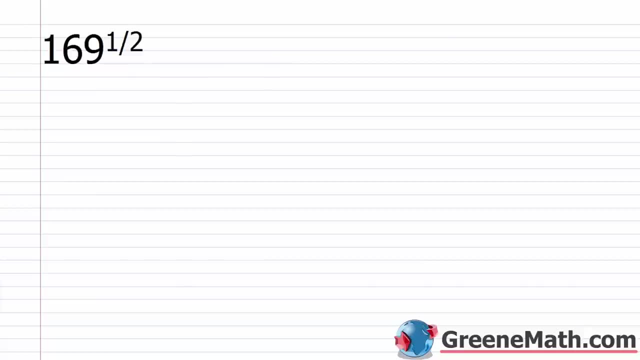 What about 169 to the power of 1 half? Again, we know this is the same as just taking the square root of the number. Raise something to the power of 1 half, like taking the square root, So I'll put: equals the square root of 169.. 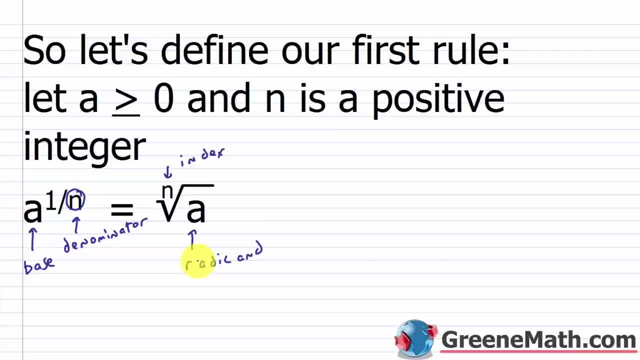 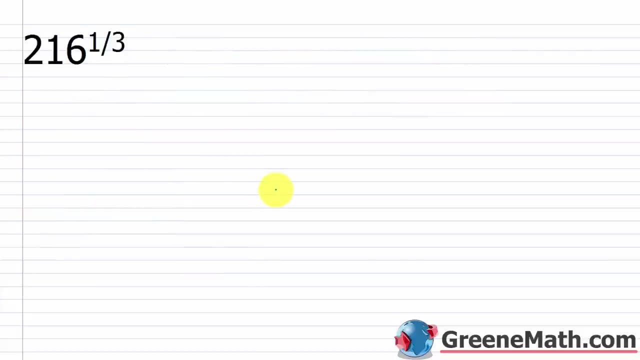 Okay. You can even do this when you're doing your practice problems or your homework. Okay. After about 10 problems or so, you're going to memorize this generic formula. And you're going to do this without having to look at that flash card. So let's start out with 216 raised to the power of one third. 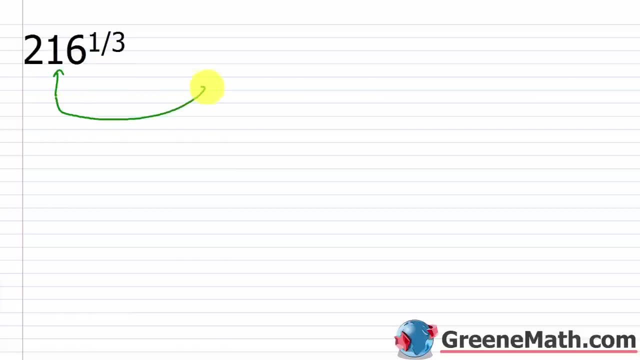 So we know that this is going to end up being our radicand okay so let me write 216 and let me write the radical and we know that 3 is going to end up being the index okay that's going to end up being the index okay again just straight from your flashcard so we end up with the cube root of 216 and most of you know at this point that that's going to be 6 all right that's going to be 6 6 times 6 is 36 36 times 6 once more is 216 what about something like 625 to the 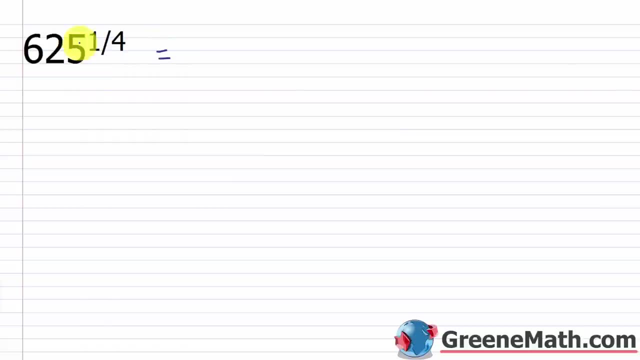 1 4th power so again this part right here would be the radicand and it would be the fourth route right because this would be your index so again this would be the index and then this would end up being the radicand so I have this as my index and this would end up being my radical so let me have the fourth root of 625. And that's equal to five, right? Five times five is 25. 25 times five 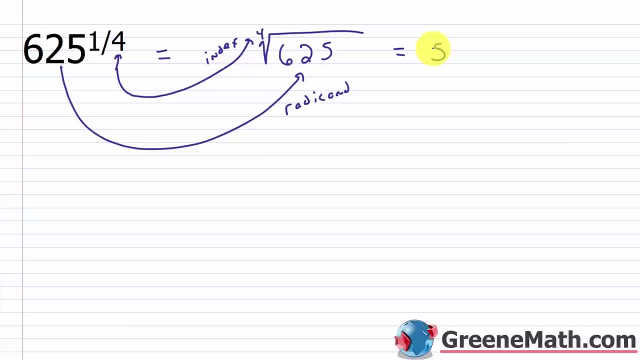 is 125. And then 125 times five is 625. What about 169 to the power of one half? Again, we know this is the same as just taking the square root of the number. Raise something to the power of one half, like taking the square root. So I'll put equals the square root of 169. And again, if you didn't 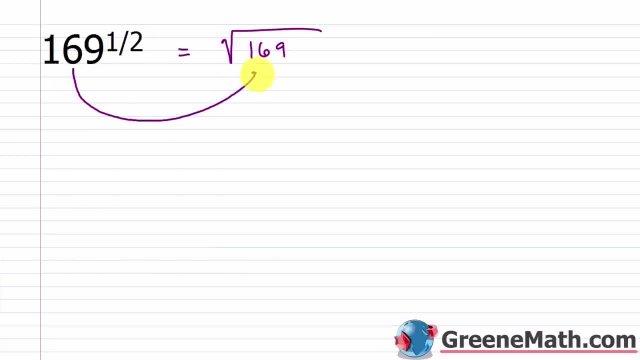 remember that, you could use the flashcard and say, okay, well, this is going to be my radicand. 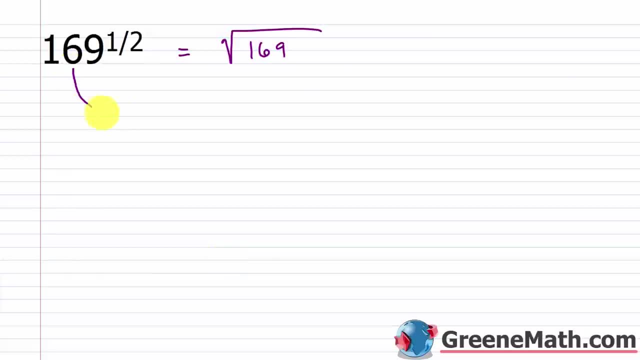 And again, if you didn't remember that, you could use the flashcard and say, okay, well, this is going to be my radicand, And then this, the denominator, is going to be my index. Now, when we work with square roots, we know that we don't display the 2, right? 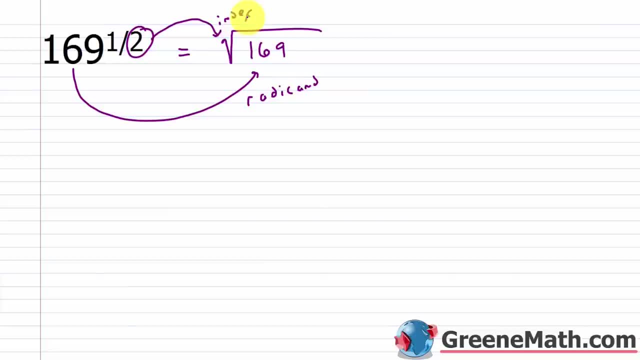 We have an understood index of a 2 when there's no index that's displayed. So we all know that the square root of 169 would be 13.. What about 243 to the 1, fifth power? Well, again, this part, right here, this 243,. 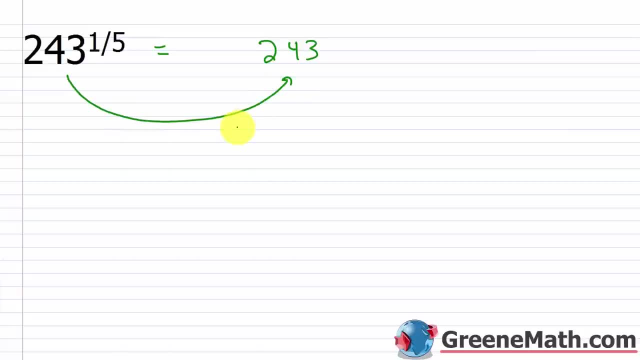 would be my radicand. Okay, this would be my radicand. And then I'm taking the fifth root of that, because this right here my denominator would be the index. Let me rewrite that. make it a little cleaner. 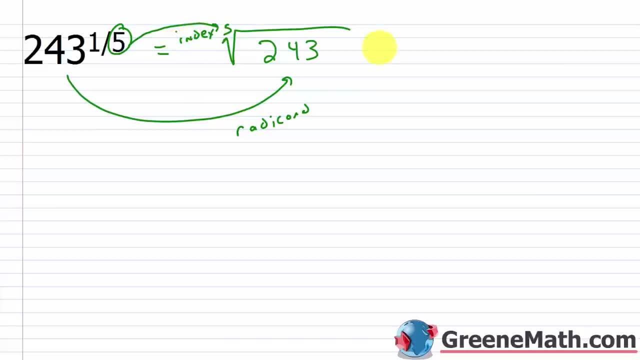 So what is the fifth root of 243?? Well, again, it's 3.. 3 times 3 is 9.. 9 times 3 is 27.. 27 times 3 is 81.. And 81 times 3 is 243.. 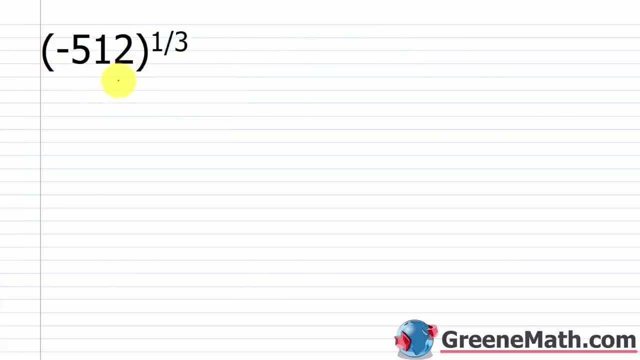 Alright, for the next one, let's look at negative 512 raised to the power of 1 third. Now, when I gave you the rule, I specifically said that this value here, which is a- and we talked about our rule- is non-negative. 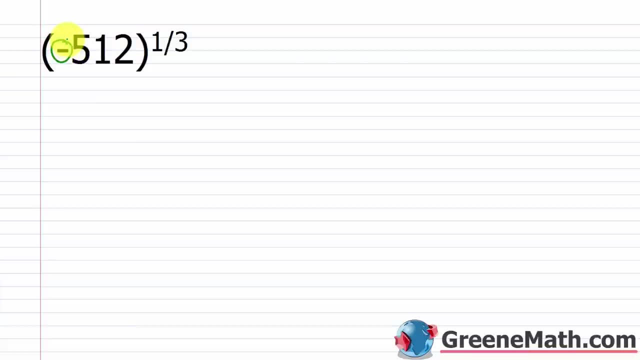 So what gives? Why is this negative? Well, I want to show you that you can also incorporate this rule with a negative. You just have to keep in mind that when you work with roots, remember you don't want to end up with a situation where you have an even index. 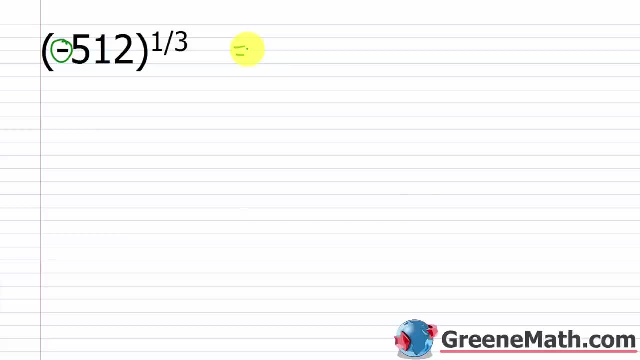 and you have a negative radicand, Alright, that's going to produce a not real solution, Okay, so we want to kind of stay away from that for right now, until we get into algebra 2, and we can kind of deal with those scenarios. 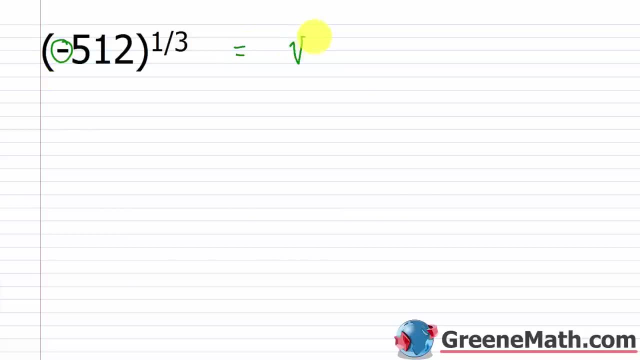 So I'm going to write the cube root, the cube root of 512, and it's negative, so I'm going to put that in there And this is okay, because the negative there when I think about a cube root. 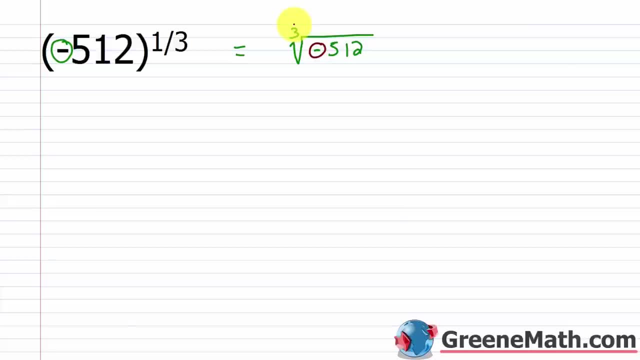 is fine, right. Negative: 1 times negative: 1 times negative: 1 is negative 1.. So I can just put a negative out in front here and then just think about 512.. What is the cube root of 512?? 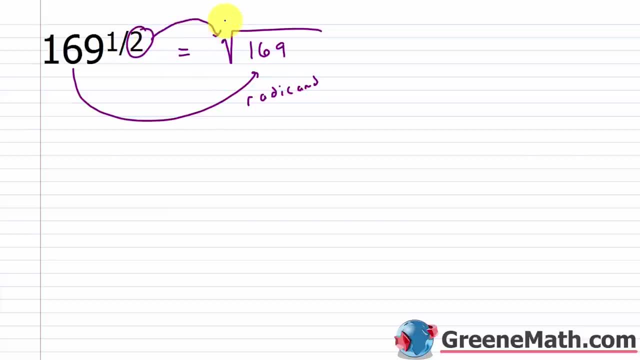 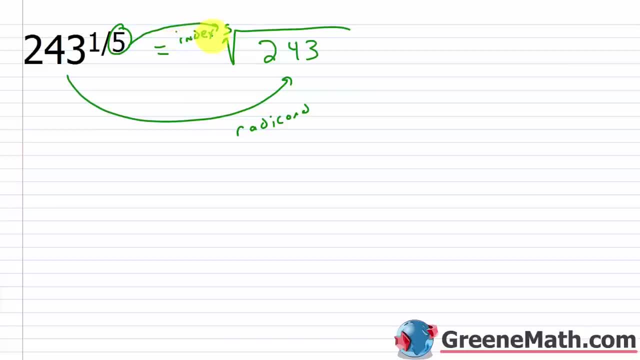 Make it a little cleaner. So what is the fifth root of 243? Well, again, it's 3. 3 times 3 is 9, 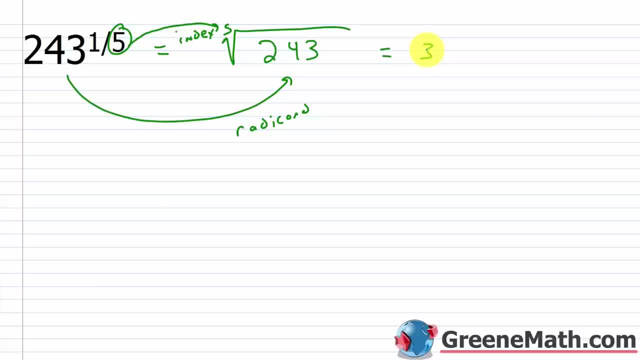 9 times 3 is 27, 27 times 3 is 81, and then 81 times 3 is 243. All right, for the next one, 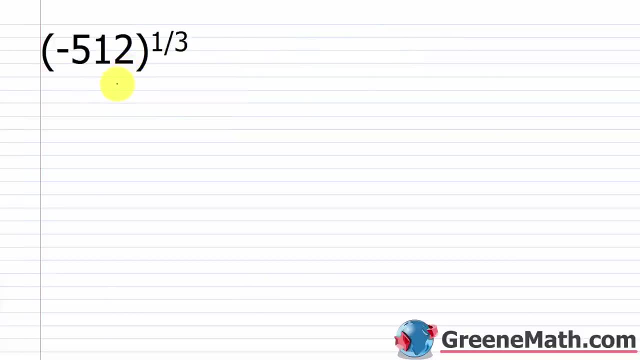 let's look at negative 512 raised to the power of one-third. Now, when I gave you the rule, I specifically said that this value here, which is a, and we talked about our rule, is non-negative. So what gives? Why is this negative? Well, I want to show you that you can also incorporate this rule with a negative. We just have to keep in mind that when you work with roots, remember, you don't want to end up with a situation where you have an even index and you have a negative radicand, right? That's going to produce a not real solution. Okay, so we want to kind of stay away from that for right now until we get into algebra two and we can kind of deal with those scenarios. 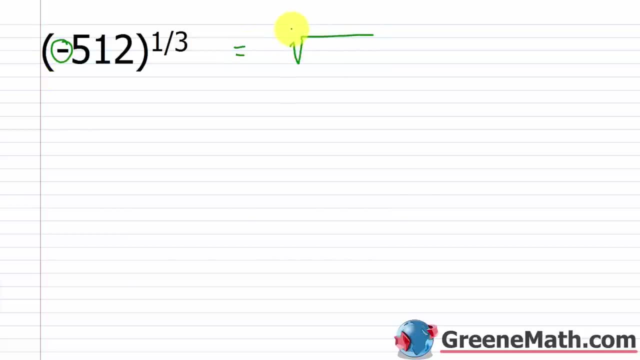 So I'm going to write the cube root, the cube root of 512, and it's negative, so I'm going to put that in there. And this is okay because the negative there, when I think about a cube root, is fine, right? Negative 1 times negative 1 times negative 1 is negative 1. So I can just put a negative out in front here and then just think about 512. What is the cube root of 512? Well, in case you don't know that, and I know up to this point I just kind of gave you the answers. Let's get a little practice in figuring this out. This ends in 12, so I know it's divisible by 4, and this would be 128 times 4. And I know that 128 is 2 to the 7th power. Some of you don't know that, so you could continue and say, okay, well, this is 64 times 2. And at this point, you should recognize 64 is 2 to the 6th power. So really, if I wrote this as 2 times 2, I could say I have 2 to the 6th power. So I could write this as 2 to the 6th power times 2 times 2 times 2. So really, this is 2 to the 6th power times 2 cubed or 2 to the 9th power. 2 to the 9th power. Now, here's where we can really kind of get things going, okay? If I have 2 to the 9th power, because that's what 512 is, forget about that negative for a second, and I took the cube root of that, how can I use what I just did, to simplify that? Well, if I realize that I'm taking the cube root, and that's like raising 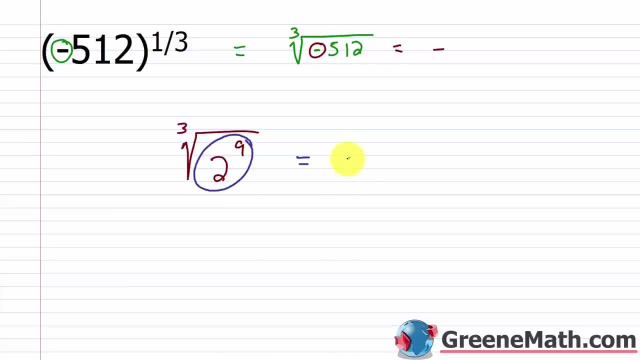 something to the 1 3rd power, I can keep this as 2 to the 9th power, and then I can raise this whole thing to the power of 1 3rd. Now, by the power rules for exponents, I know that I would multiply. This is like saying I have 2 to the power of what? 9 times 1 3rd is 9. Which is really equal to 2 to the power of 3 or 8. So this is going to equal negative 8. And the reason I did this this way is because it's going to lead into what we're going to do next, okay? I 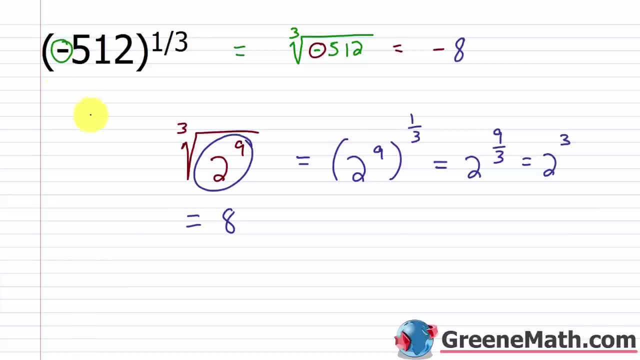 wanted to give you a brief example. So negative 512 raised to the 1 3rd power is negative 8. 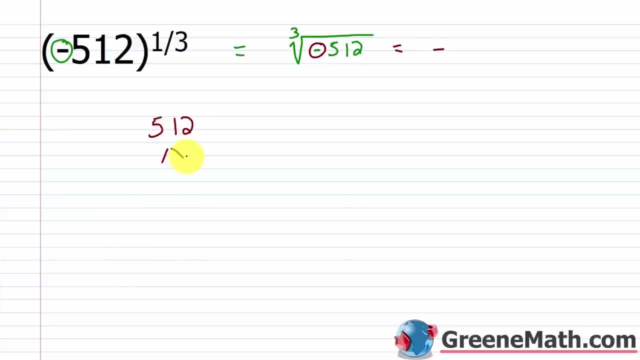 Well, in case you don't know that- and I know up to this point- I just kind of gave you the answers. let's get a little practice in figuring this out. This ends in 12, so I know it's divisible by 4,. 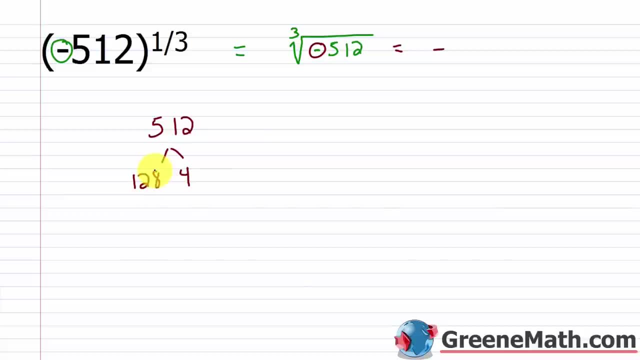 and this would be 128 times 4.. And I know that 128 is 2 to the 7th power. Some of you don't know that, so you can continue and say: okay, well, this is 64 times 2,. 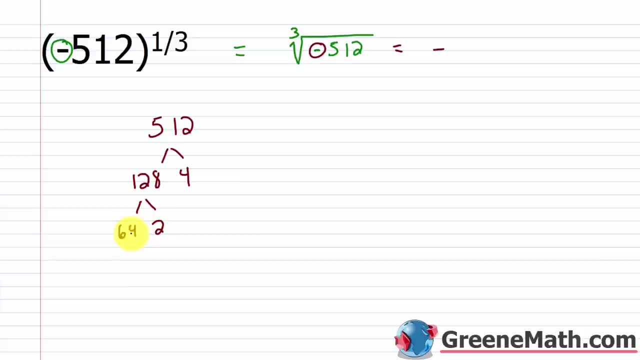 and at this point you should recognize: 64 is 2 to the 6th power. So really, if I wrote this as 2 times 2, I could say I have 2 to the 6th power times 2 times 2 times 2.. 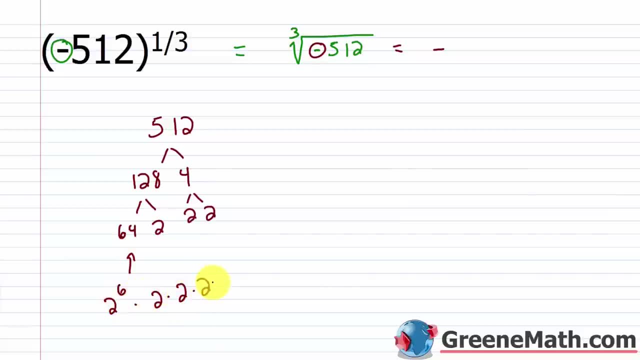 So really, this is 2 to the 6th power, times 2 cubed, or 2 to the 9th power, 2 to the 9th power. Now here's where we can really kind of get things going okay. 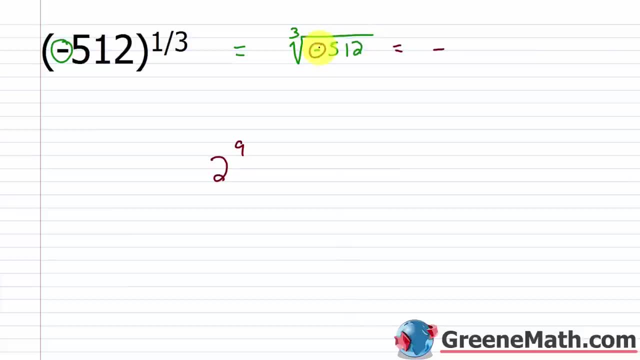 If I have 2 to the 9th power, because that's what 512 is, forget about that negative for a second. and I took the cube root of that. how can I use what I just did to simplify that? Well, if I realize, if I realize that I'm taking the cube root, 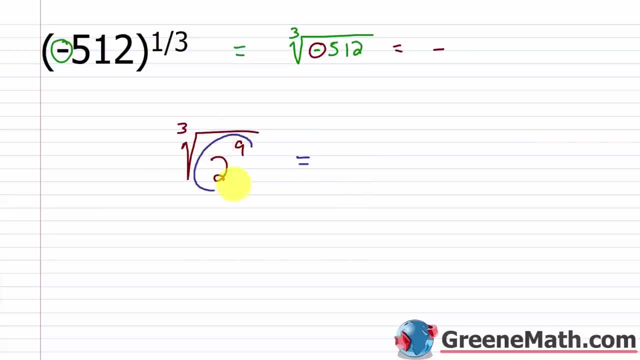 and that's like raising something to the 1- 3rd power. I can keep this as 2 to the 9th power and then I can raise this whole thing to the power of 1- 3rd. Now, by the power rules for exponents. 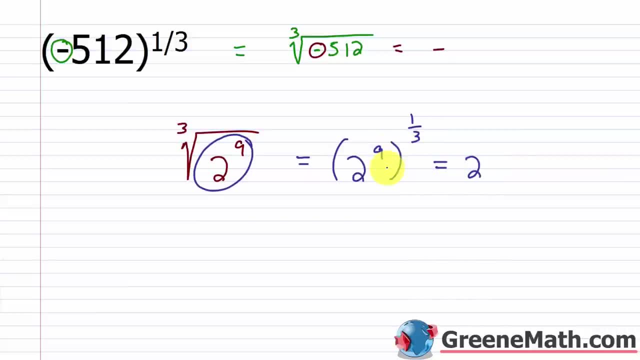 I know that I would multiply. This is like saying I have 2 to the power of what. 9 times 1, 3rd is 9 3rds, which is really equal to 2 to the power of 3,. 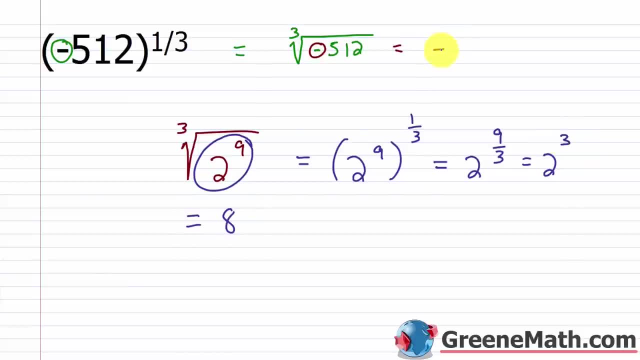 or 8.. So this is going to equal negative 8. And the reason I did this this way is because it's going to lead into what we're going to do next. okay, I wanted to give you a brief example. So negative 512 raised to the 1- 3rd power is negative 8.. 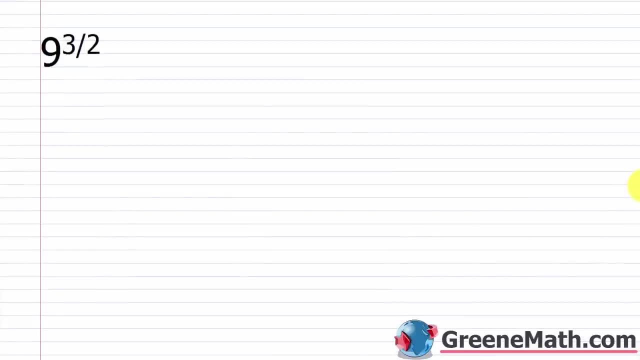 So what would I do in a scenario where I have 9 to the power of 3 halves? Well, just like in the last example, I'm able to kind of break this up using my power rules for exponents. So what I can do, 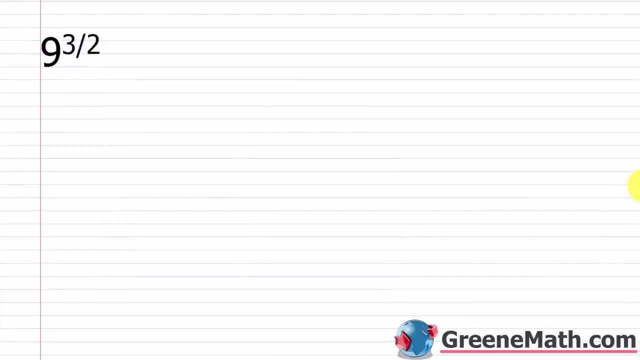 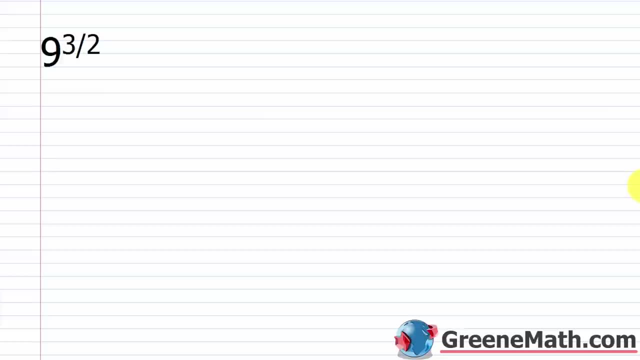 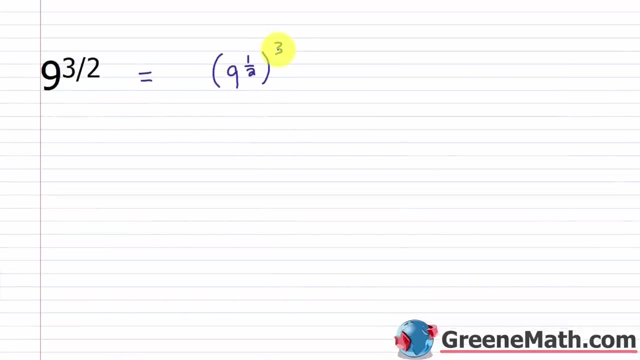 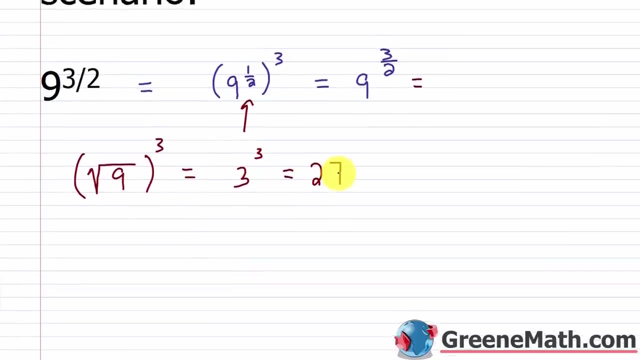 So I'm going to have 9 to the power of 3 halves. So I'm able to kind of break this up using my power rules for exponents. So what I can do, I'm just going to look at this for a second. I can rewrite this as 9 to the power of 1 half, and then this is going to be raised to the 3rd power. And again, if you use the power rules for exponents, you'll see that you end up with the same thing. I'd multiply the exponents here and keep the base the same. This is equal to 9 raised to the power of 3 over 2. So I can go back and forth. But the reason I would want to write it like this is because it makes it obvious what I need to do. I know that 9 to the power of 1 half, at this point in your mind, might still not register as the square root of 9. It does for me, but I've been doing this for a long time. So you might want to say, okay, this is the square root of 9, just following the processes we've been doing, right? 9 is the radicand, the index. Then, once I've written it like that, I can raise this to the 3rd power, and then it's completely crystal clear that this is 3, right? Square root of 9 is 3. That's raised to the 3rd power, or 3 cubed, which gives us a final answer here of 27. All right, let's try another one. 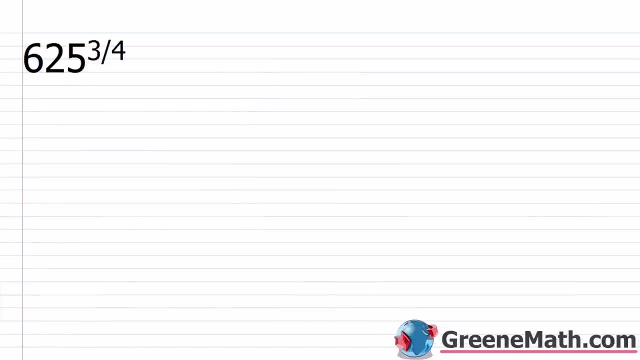 We have 625 raised to the 3 4ths power. Again, I'm going to break this up, 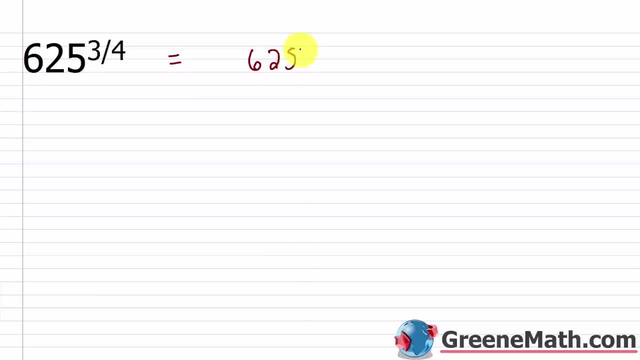 and I'm going to think about this as 625 raised to the power of 1 4th. And then I'm going to cube this. And again, I'm going to write this, thinking about this as the 4th root of 625. Again, this is the radicand, so that comes down here. 4 is the index. And then 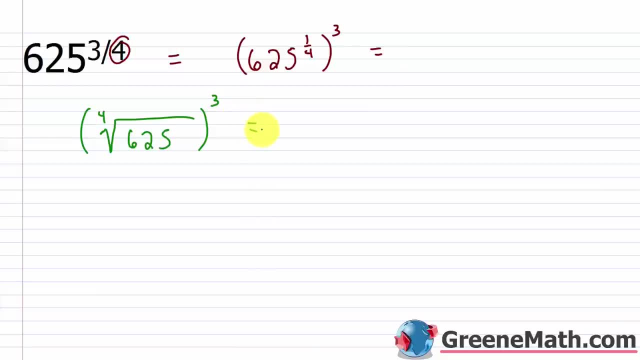 I'm going to cube this guy. So what is the 4th root of 625? I talked about that earlier. It's 5. 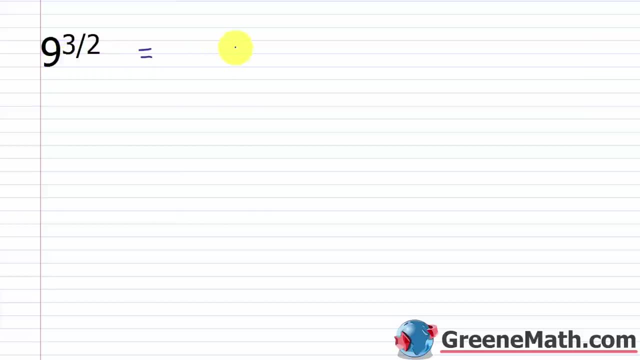 and just kind of look at this for a second, I can rewrite this as 9 to the power of 1 half, and then this is going to be raised to the 3rd power. And again, if you use the power rules for exponents, 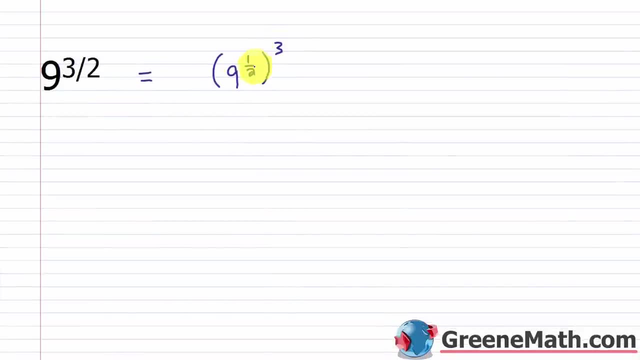 you'll see that you end up with the same thing. I'd multiply the exponents here and keep the base the same. This is equal to 9 raised to the power of 3 over 2, right, So I can go back and forth. 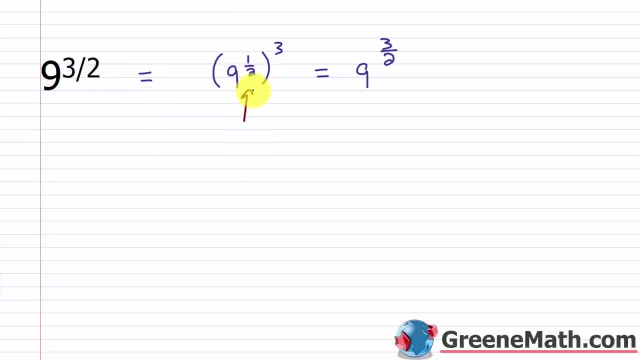 But the reason I would want to write it like this is because it makes it obvious what I need to do. right, I know that 9 to the power of 1 half at this point in your mind might still not register as the square root of naught. 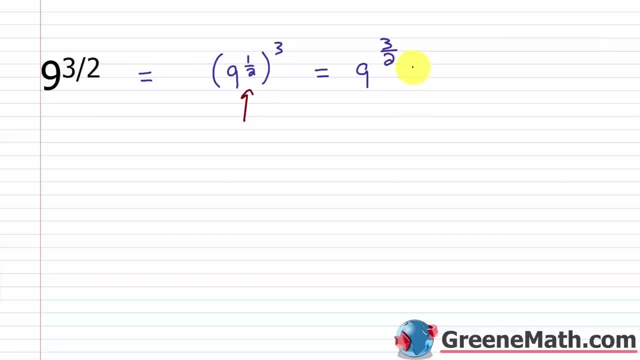 It does for me, but I've been doing this for a long time, So you might want to say: okay, this is the square root of 9, just following the processes we've been doing right. 9 is the radicand, 2 is the index. 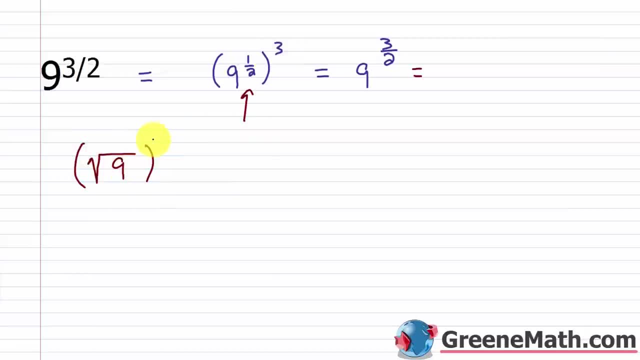 Then, once I've written it like that, I can raise this to the 3rd power, And then it's completely crystal clear that this is 3, right Square root of 9 is 3.. That's raised to the 3rd power, or 3 cubed. 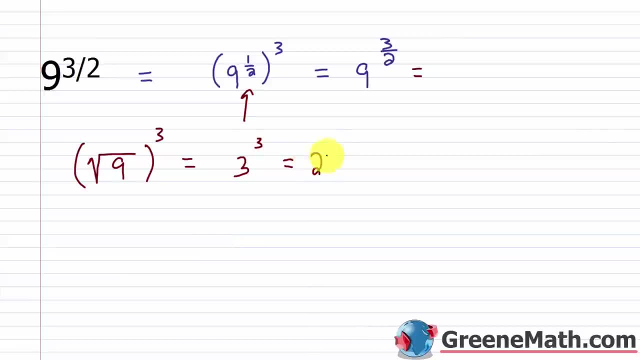 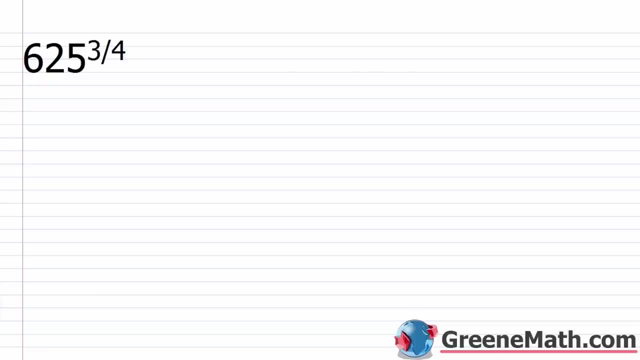 which gives us a final answer here of 27.. Alright, let's try another one. We have 625 raised to the 3 fourths power. Again, I'm going to break this up and I'm going to think about this as. 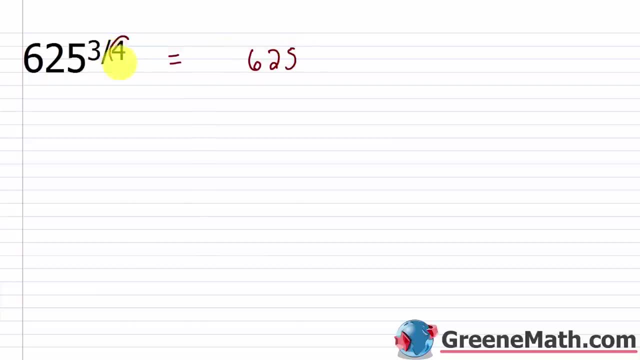 625 raised to the power of 1 fourth. and then I'm going to cube this And again I'm going to write this, thinking about this as the 4th root of 625.. Again, this is the radicand. 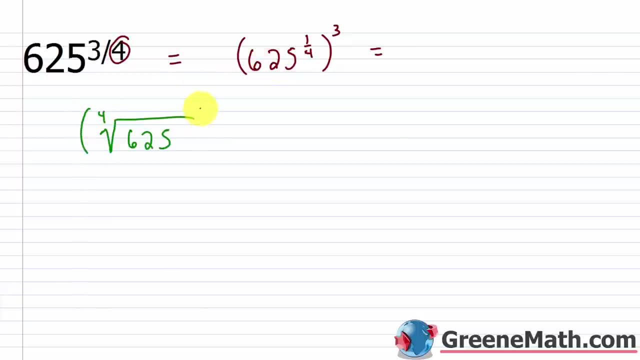 so that comes down here. 4 is the index, And then I'm going to cube this guy. So what is the 4th root of 625? Talked about that earlier, it's 5.. So this would basically just be what. 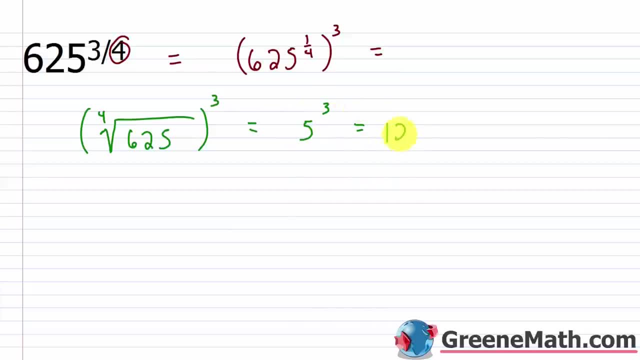 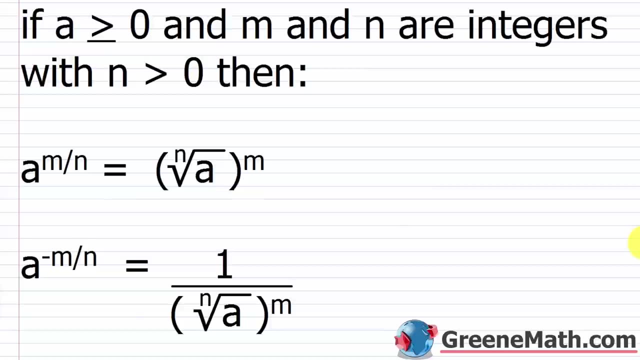 It'd be 5 cubed, which is 125.. Alright, so now let's look at the more tedious rule. You definitely want to write this down, because this is one that takes a little bit longer to get down. So, if a is greater than or equal to 0,. 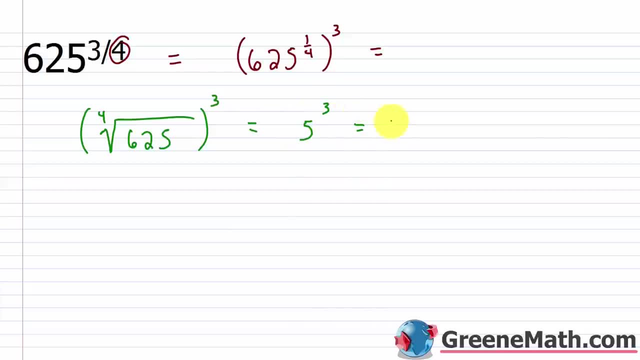 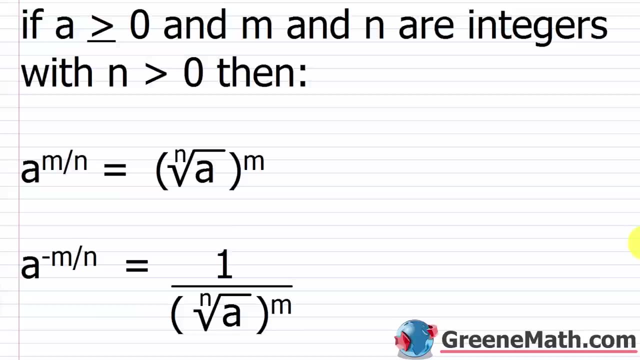 Basically, it'd just be what? It'd be 5 cubed, which is 125. All right, so now let's look at the more tedious rule. You definitely want to write this down, because this is one that takes a little 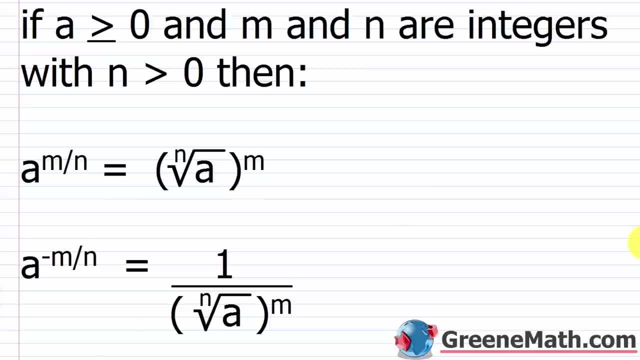 bit longer to get down. So if a is greater than or equal to 0, so again, if a is non-negative, and m and n are integers with n greater than 0, okay? So n is greater than 0 because we want it to be positive. So then we have this scenario. 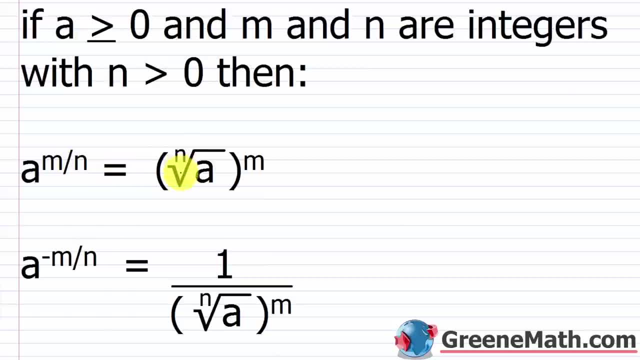 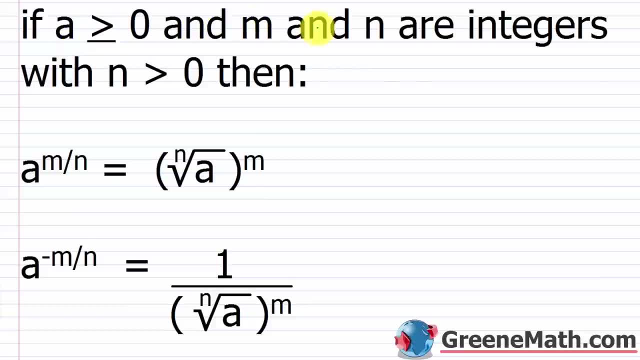 so again, if a is non-negative and m and n are integers with n greater than 0. So n is greater than 0 because we want it to be positive. So then we have this scenario: a raised to the power of m over n. 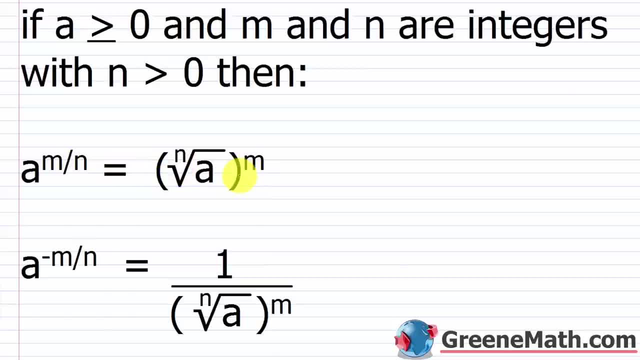 is equal to the nth root of a and this is raised to the power of m. This is what we just did. Don't let these letters confuse you. If I was to write this as 9 to the power of 3 halves. 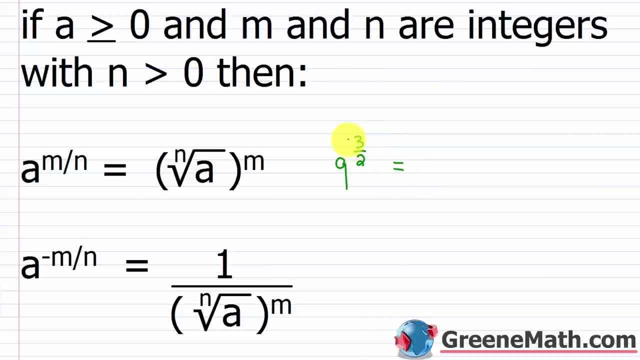 just like we just did. all I did was 3 in this case is m, So 3 is going to go on the outside. n is 2 in this case, so it's going to be the square root of alright. that's my index. 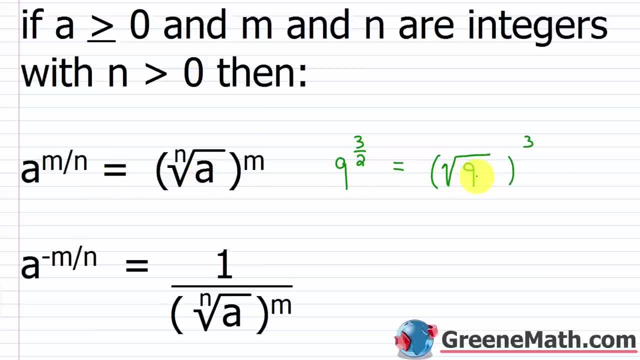 and the a in this case is just the radicand, it's 9.. It's the same thing. So again, if you struggle with generic formulas like this, write it down and then, before you do anything on each problem. 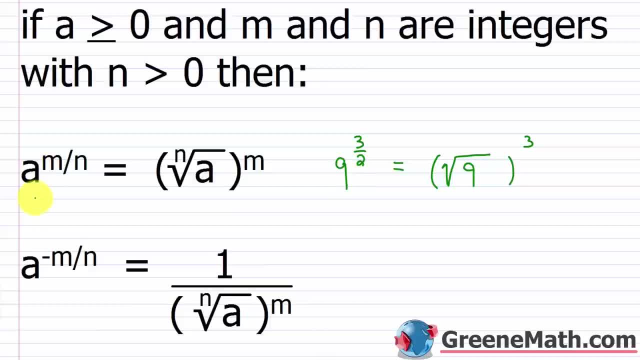 just say: okay, my a here is 9.. Write a 9.. Write a 9 underneath. My m here is 3.. Write a 3 there. My n here is 2.. Write a 2 there And then just translate it into this formula here: 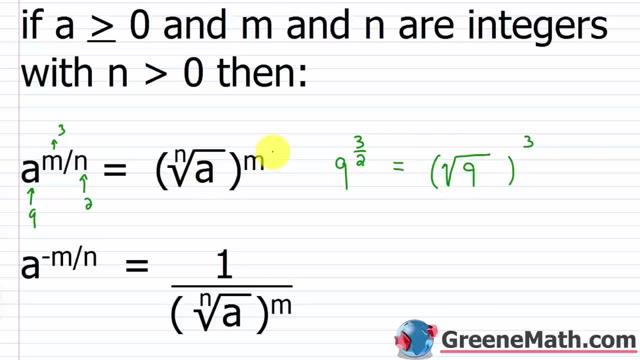 I have a 2 here, I have a 9 here and I have a 3 here. Once you start doing that over and, over and over again, this becomes really, really easy, Okay, So, especially if you struggle with these formulas, 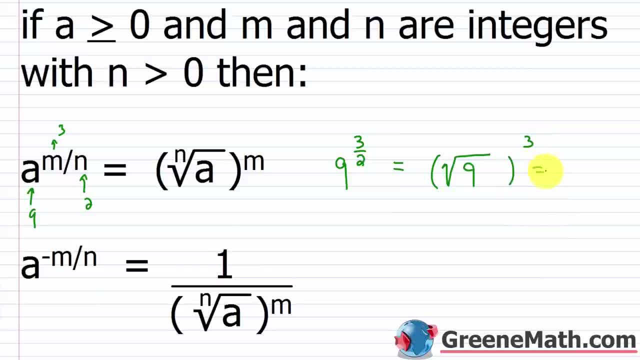 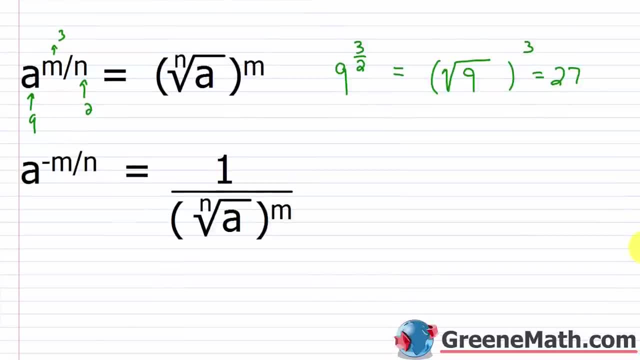 please do that every time Now, for completeness sake. we know the answer to this: square root of 9 is 3, 3 cubed is 27.. Now here's one you probably have not seen yet. So we have a raised to the power of a negative m. 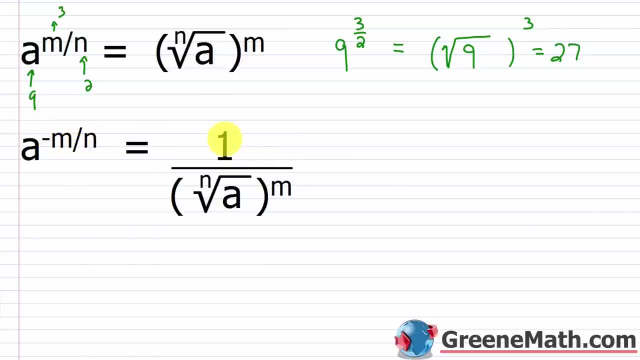 over n. So we have this is equal to 1 over. we have the nth root of a and this is raised to the power of m. There's no difference between this formula and this formula, other than we just take the reciprocal. 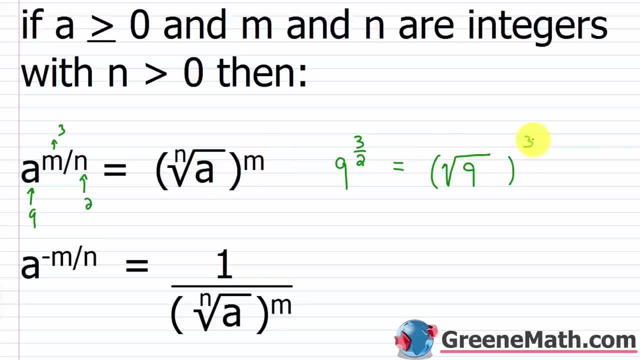 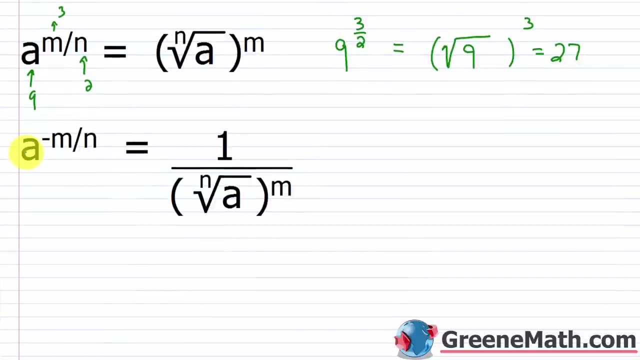 And I have a 3 here. Once you start doing that over and over and over again, this becomes really, really easy. Okay? So especially if you struggle with these formulas, please do that every time. Now, for completeness sake, we know the answer to this. Square root of 9 is 3. 3 cubed is 27. Now, here's one you probably have not seen yet. So we have a raised to the power of a negative m over n. So we have this. 1 over, we have the nth root of a, and this is raised to the power of m. There's no difference between this formula and this formula, other than we just take the reciprocal. We take the reciprocal of this guy, okay? And we raise it to this guy being positive. It's just like when we saw 2 to the power of negative 4. We took the reciprocal of the base, and we made the exponent positive. So really, to make this crystal clear, I could say, okay, I have a 2 to the power of negative m over n. I could write this as 1 over a to the power of m over n, right? All I did was, I took the reciprocal of the base, so I have 1 over a, and then the exponent just became positive. 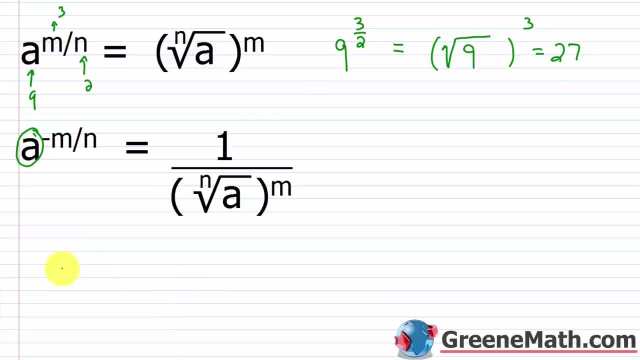 Instead of negative m, it's positive m. As an example of this, let's say I saw something like 27 raised to the power of negative 2 thirds. So following this, 27 represents a, the negative 2, the whole thing, is representing the negative m. Or you could say 2 represents m, and you have a negative out in front, however you want to think about that. 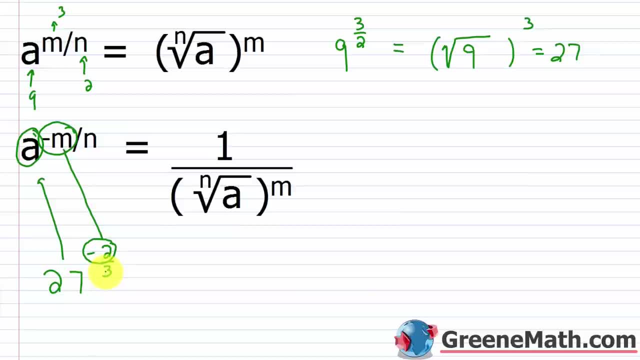 Then n represents 3, okay? So if I translate this over here, I would basically have what? I'd have 1 over 27 raised to the power of 2 thirds. And then if I said I had 1 over the cube root of 27, and then this guy would be squared, I'd end up with a final answer of one over the cube root of 27 is three. So it'd be three squared, which is nine. So I'd end up with one ninth in that scenario. The key to this is just to write down the generic formulas, match things up and just 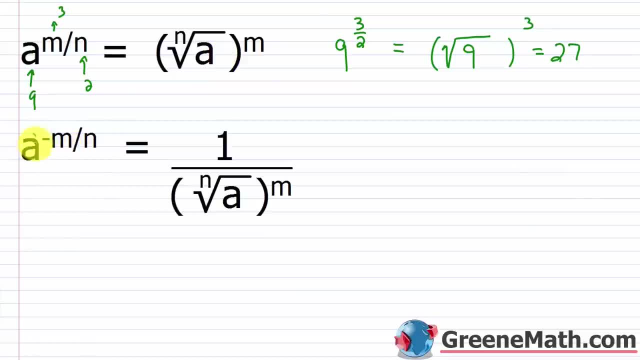 we take the reciprocal of this guy okay and we raise it to this guy being positive. It's just like when we saw 2 to the power of negative 4, we took the reciprocal of the base and we made the exponent positive. 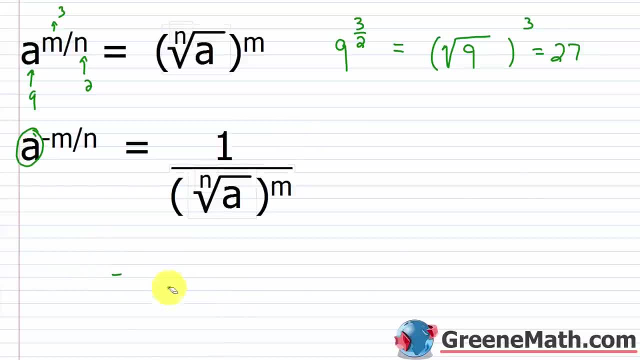 So really to make this crystal clear, I could say: if I have a to the power of negative m over n, I could write this as 1 over a to the power of m over n. right, All I did was I took the reciprocal of the base. 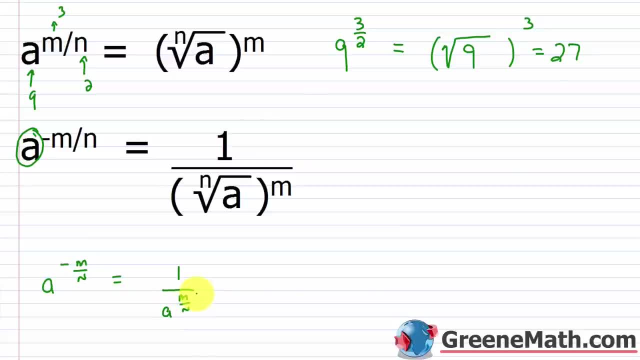 so I have 1 over a, and then the exponent just became positive. Instead of negative m, it's positive m. As an example of this, let's say, I saw something like 27 raised to the power of negative 2 thirds. 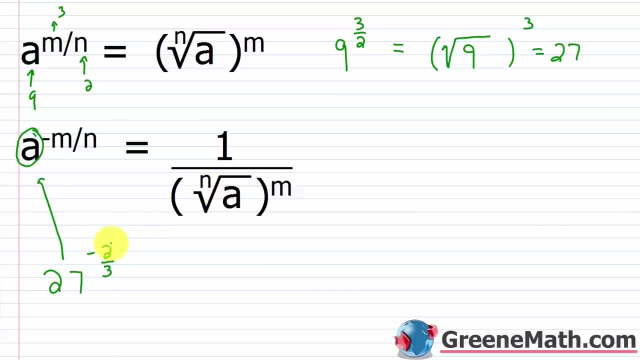 So, following this, 27 represents a, the negative 2, the whole thing is representing the negative m. Or you could say 2 represents m and you have a negative out in front. however you want to think about that, Then n represents 3,. 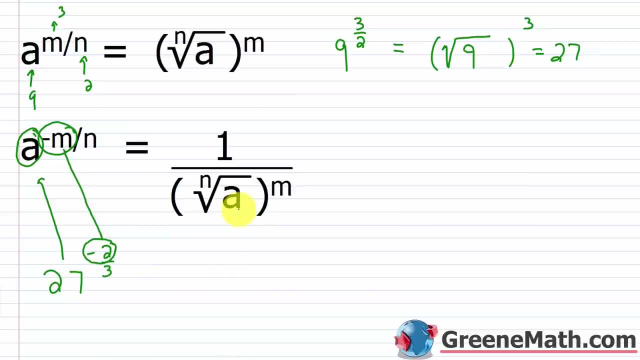 okay. So if I translate this over here, I would basically have what I'd have: 1 over 27 raised to the power of 2 thirds, And then if I said I had 1 over the cube root of 27, and then this guy would be squared. 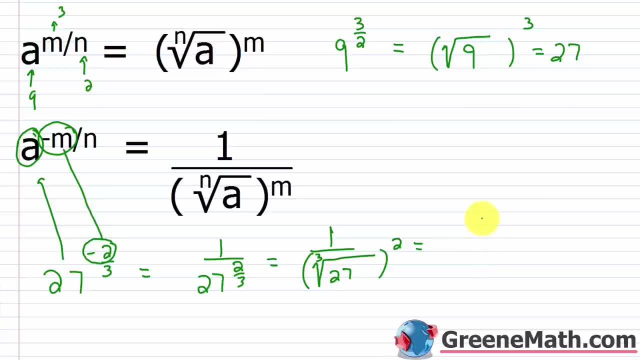 I'd end up with a final answer of 1 over the cube. root of 27 is 3.. So it'd be 3 squared, which is 9, so I'd end up with 1, ninth, in that scenario. The key to this is just to write down the generic formulas. 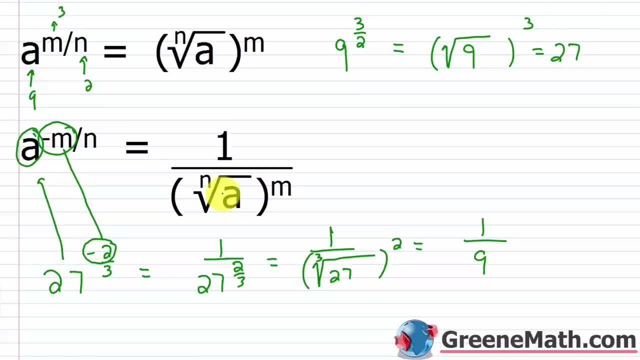 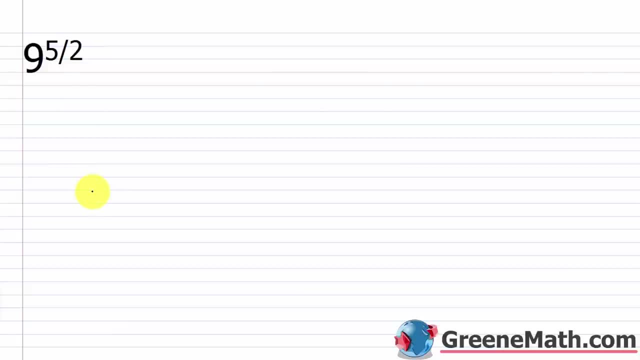 match things up and just go slowly right, Just take it step by step. All right, what if we saw 9 to the power of 5 halves? Again, I'm going to break this up. I'm going to say: this is a square root of 27,. 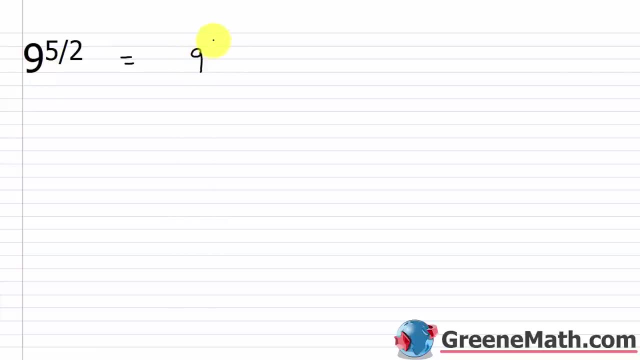 so I'm going to say this is 9 to the power of 1 half, and this is raised to the 5th power, And again, this would be the square root of 9 raised to the 5th power, which is what. 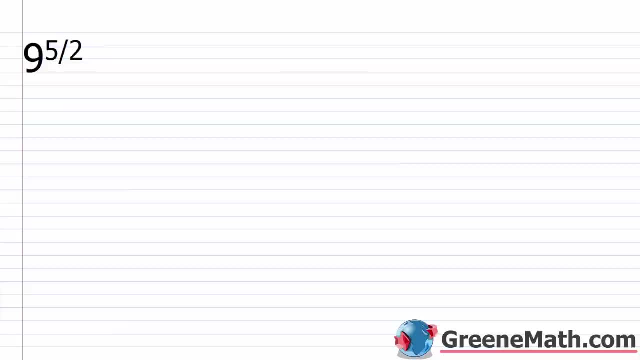 go slowly, right? Just take it step by step. All right. What if we saw nine to the power of five halves? Again, I'm going to break this up. I'm going to say this is nine to the power of one 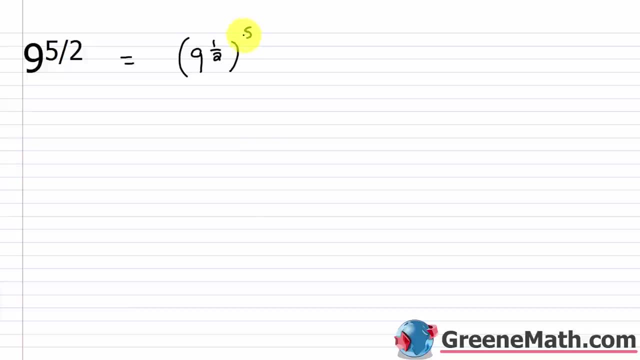 half, and this is raised to the fifth power. And again, this would be the square root of nine raised to the fifth power, which is what? Three to the fifth power, which is 243. 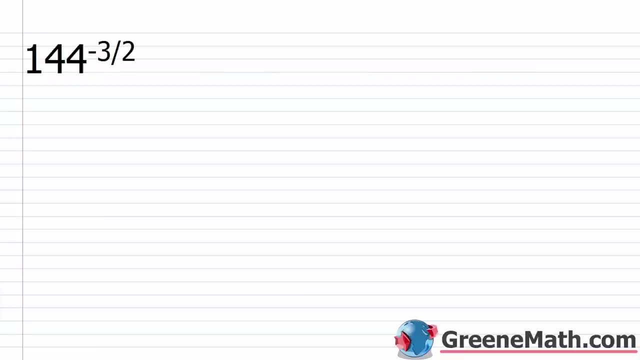 What about 144 raised to the power of negative three halves? Again, take the reciprocal of the base. So take the reciprocal of the base, which is three to the power of nine, which is 243. 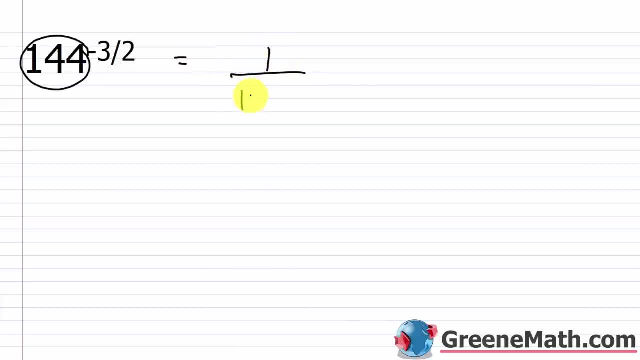 Take the reciprocal of 144, that's just one over 144, and then raise it to the power of three halves. Exponent's just going to become positive, okay? Just that simple. So then I break this up. I have one over, this is 144 raised to the one half power, and then it's cubed. So I'm going to write this as one over the square root of 144, and then that's going to be one over 144. 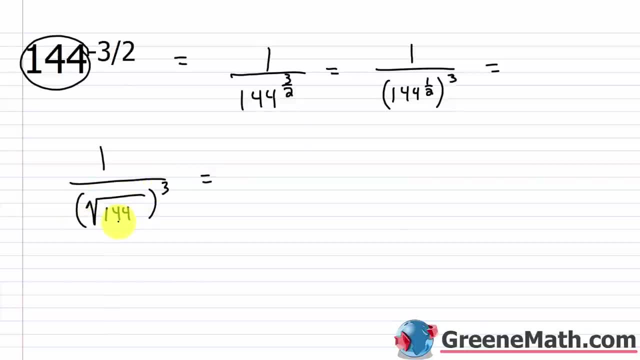 So this is going to be cubed. And so the square root of 144 is 12. So this ends up being one over 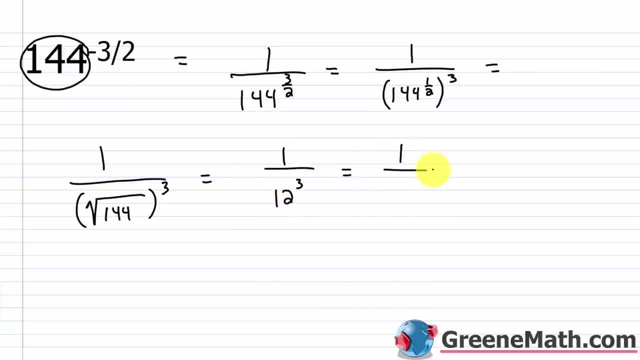 12 cubed, which is one over 1,728. What about negative 128 raised to the power of eight sevenths? 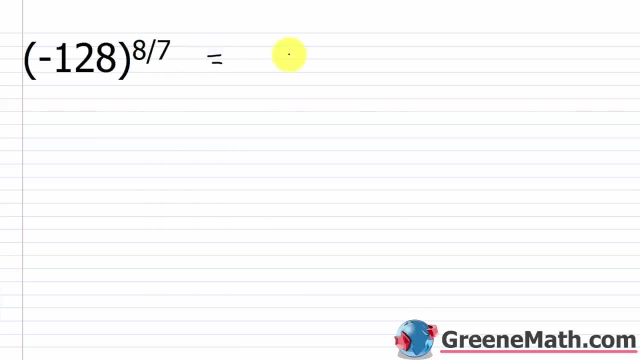 So again, I can break this up and say this is negative 128. Now this is inside of parentheses. 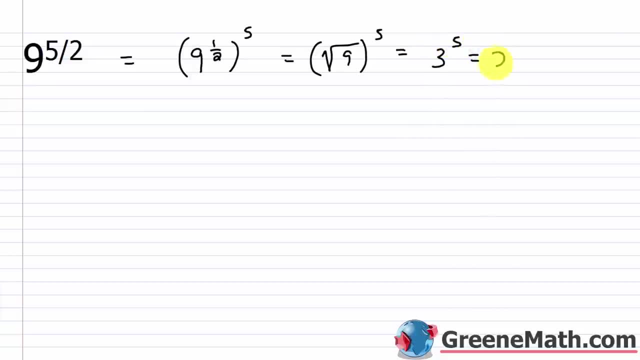 3 to the 5th power, which is 243.. What about 144? raised to the power of negative, 3 halves Again. take the reciprocal of the base, So take the reciprocal of 144, that's just 1 over 144,. 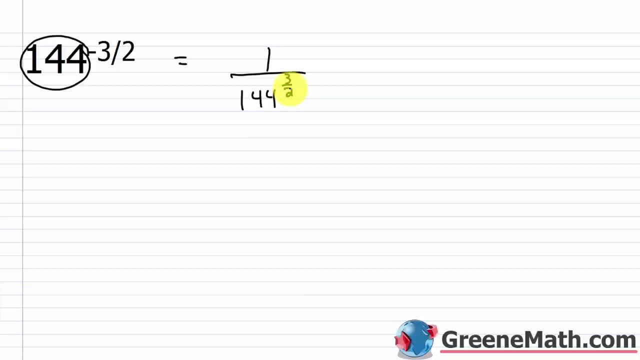 and then raise it to the power of 3 halves, The exponent is just going to become positive. okay, Just that simple. So then I break this up. I have 1 over. this is 144 raised to the 1 half power. 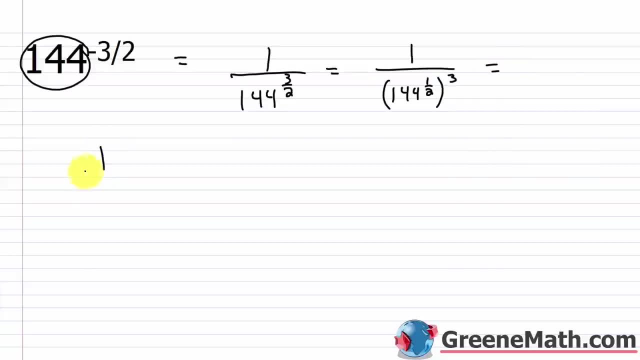 and then it's cubed. So I'm going to write this as 1 over the square root of 144, and then that's going to be cubed, And so the square root of 144 is 12, so this ends up being 1 over 12 cubed. 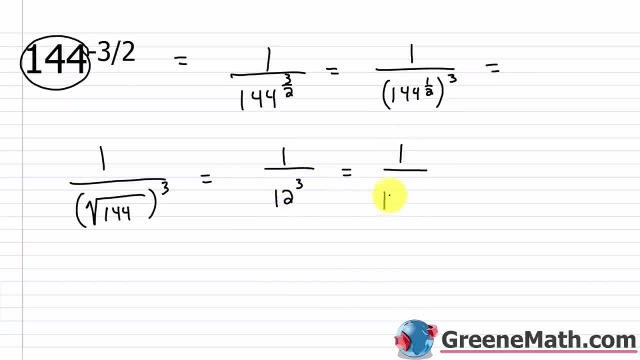 which is 1 over 1,728.. What about negative 128 raised to the power of 8 sevenths? So again, I can break this up and say this is negative 128.. Now, this is inside of parentheses. so this guy is going to be raised to the power of. 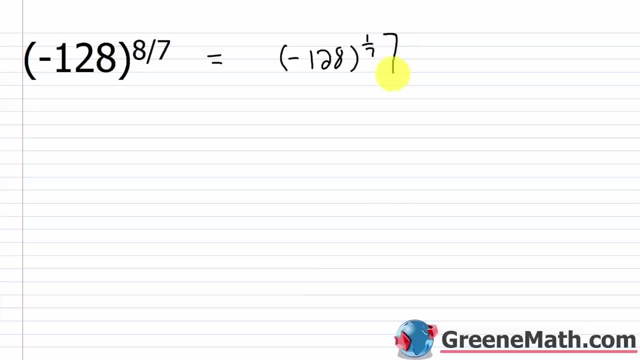 what? 1 seventh, and then I'm going to raise the whole thing. let me just use brackets here- to the eighth power, And then let me write it in a better way for you to where it's more familiar. This would be the radicand. 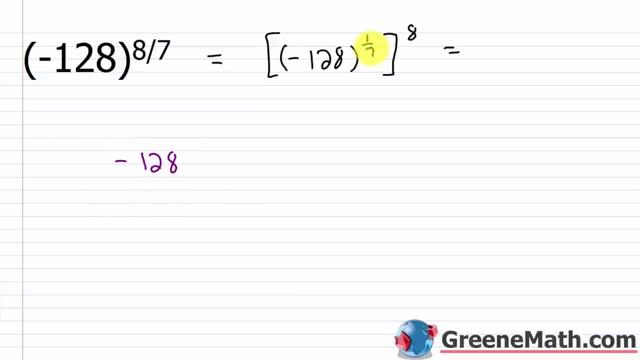 the negative 128, and I would have the seventh root, because that's my denominator, and this whole thing would be raised to the eighth power. Now we know that the seventh root of negative 128 is negative 2.. So again, 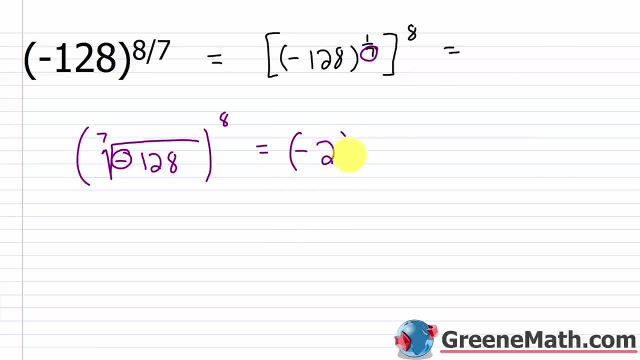 negative 2 is the result there. And then this is still inside of parentheses here and it's raised to the eighth power. So when we raise it to the eighth power, we're going to end up with 256.. And again, because this negative is inside of parentheses. 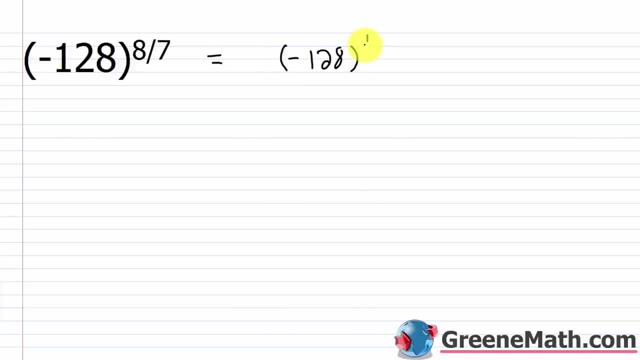 So this guy is going to be raised to the power of eight sevenths. So this guy is going to be raised to the power of one seventh. And then I'm going to raise the whole thing, let me just use brackets here, to the eighth power. And then let me write it in a better way for you, to where it's more familiar. This would be the radicand, the negative 128. And I would have the seventh root, because that's my denominator. And this whole thing would be raised to the eighth power. Now, we know that the seventh root of negative 128 is negative two. So again, negative two is the result there. And then this is still inside of parentheses here. And it's raised to the eighth power. So when we raise it to the eighth power, we're going to end up with 256. And again, because this negative is inside of parentheses, this would end up being positive 256. All right, now let's look at a few with some variables involved. The same rules apply. 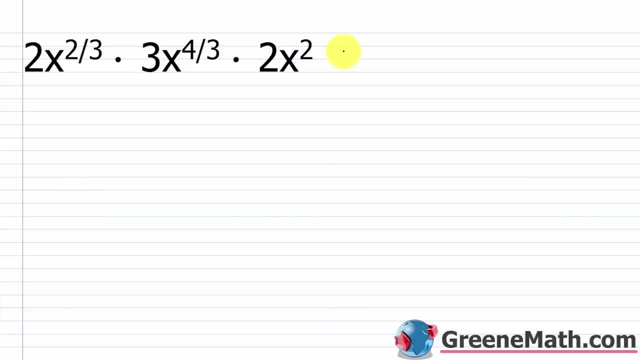 Okay, just because you're working with variables doesn't mean it got more difficult. All right, so I have 2x to the power of two thirds, times 3x to the power of four thirds, times 2x squared. Now, we know what to do here. We're going to multiply the coefficients together. 2 times 3 is 6. 6 times 2 is 12. 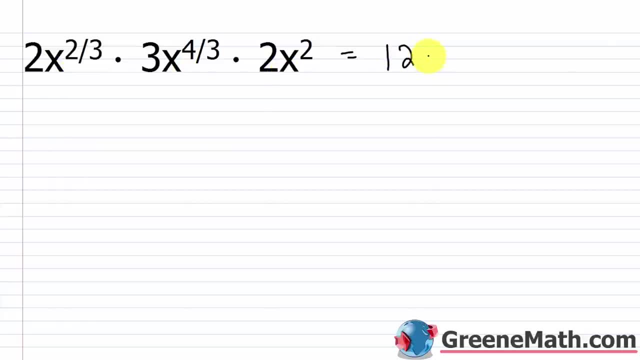 Then we have x in each case. So it's the same base. We're going to add the exponents. So I have an exponent of 12. And then I'm going to add the exponents. So I have an exponent of 12. 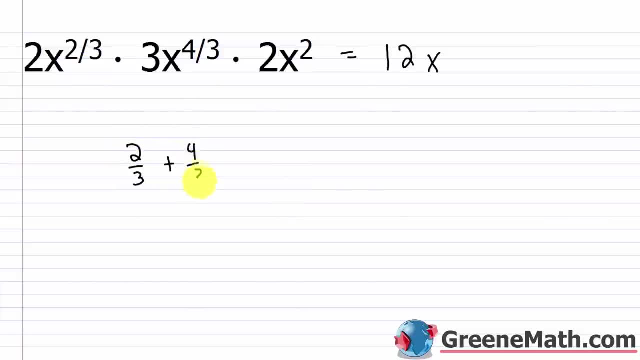 So I have 2 thirds, an exponent of 4 thirds, and an exponent of 2, which to get a common denominator, I'm going to write as 6 thirds. 2 plus 4 is 6. 6 plus 6 is 12. So this is 12 thirds, which equals 4. So my exponent on x would end up being a 4. So I end up with what? 12x to the fourth power 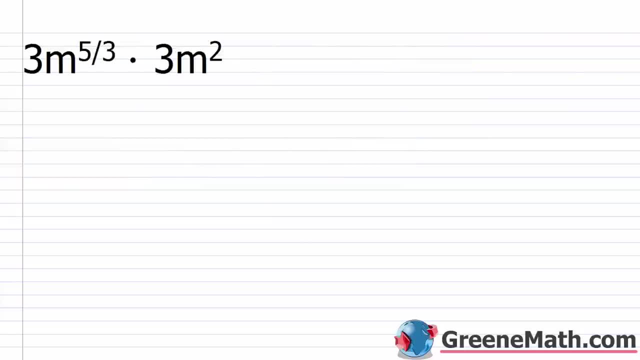 as my answer. What about something like 3m to the 5 thirds? 3m to the 5 thirds power times 3m squared. 3 times 3 is 9. And then m to the 5 thirds power times m squared. So we know m stays the same. We just have 5 thirds plus 2. So I can write 2 is 6 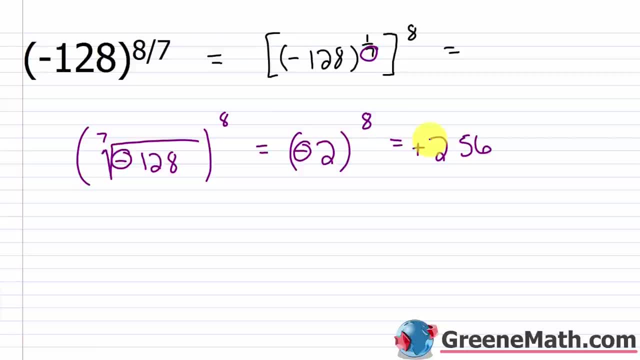 this would end up being positive 256.. All right, now let's look at a few with some variables involved. The same rules apply. Okay, just because you're working with variables doesn't mean it got more difficult. All right, so I have 2x to the power of 2 thirds. 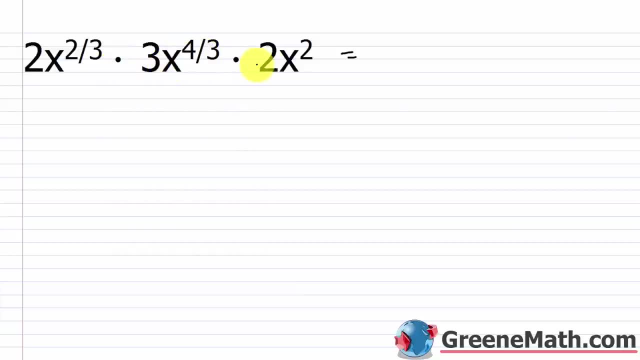 times 3x to the power of 4 thirds times 2x squared. Now we know what to do here. We're going to multiply the coefficients together: 2 times 3 is 6,. 6 times 2 is 12.. 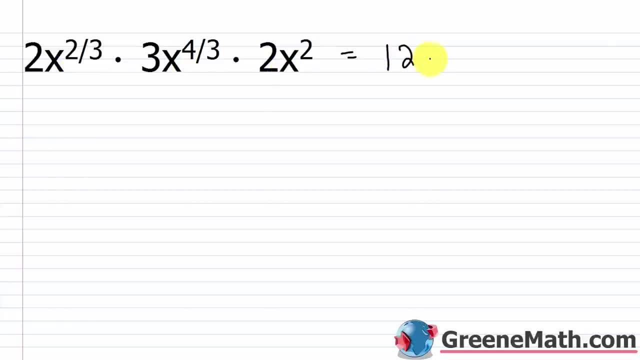 Then we have x in each case, So it's the same base. We're going to add the exponents, So I have an exponent of 2 thirds, an exponent of 4 thirds and an exponent of 2, which to get a common denominator. 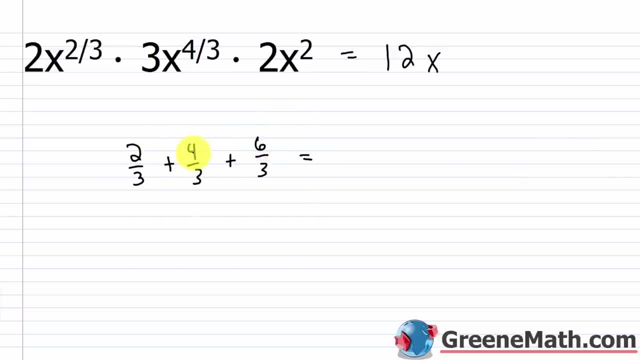 I'm going to write as 6 thirds. 2 plus 4 is 6.. 6 plus 6 is 12.. So this is 12 thirds, which equals 4.. So my exponent on x would end up being a 4.. 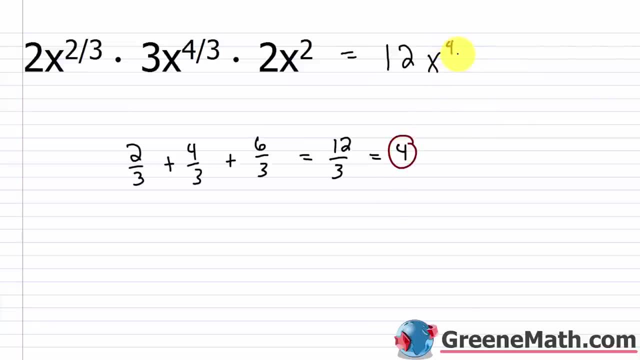 So I end up with what? 12x to the fourth power as my answer. What about something like 3m to the 5 thirds power times 3m squared 3 times 3 is 9.. And then m to the 5 thirds power. 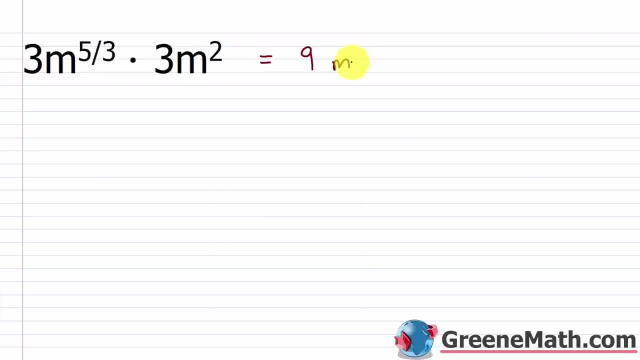 times m squared. So we know m stays the same. We just have 5 thirds plus 2.. So I can write: 2 is 6 thirds, So this ends up being 11 thirds. So 11 thirds, All right. 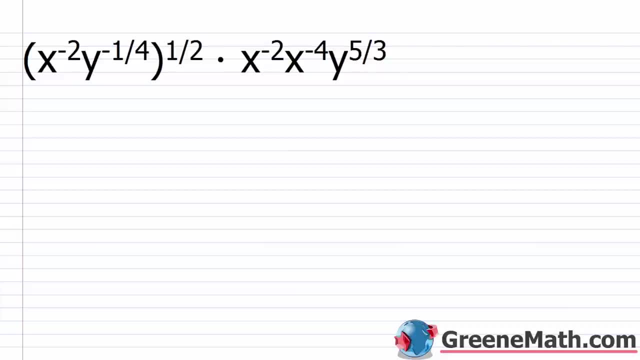 what about this one? We have x to the power of negative 2, times y to the power of negative 1. fourth, And this is raised to the 1 half power. Then we're multiplying by x to the power of negative 2,. 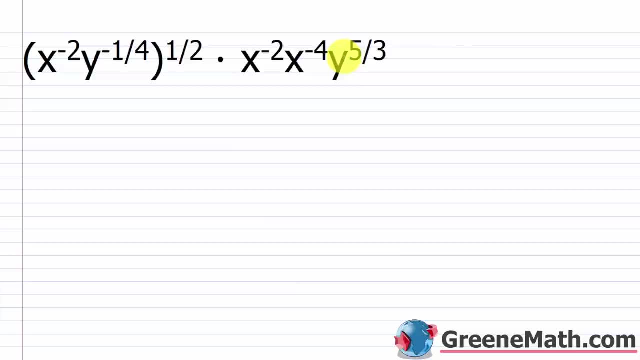 times x to the power of negative 4, times y to the 5 thirds power. So the first thing I want to do is use my power rule here. So x stays the same in this scenario And we have negative 2 raised to the 1 half power. 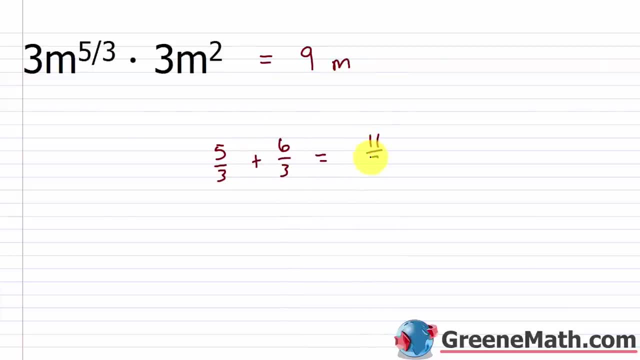 thirds. So this ends up being 11 thirds. So 11 thirds. All right, what about this one? We have 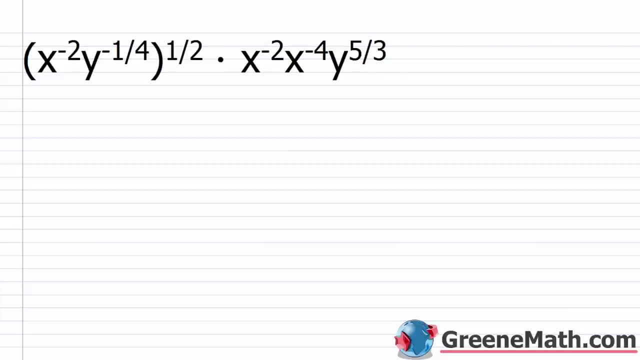 x to the power of negative 2 times y to the power of negative 1 fourth. 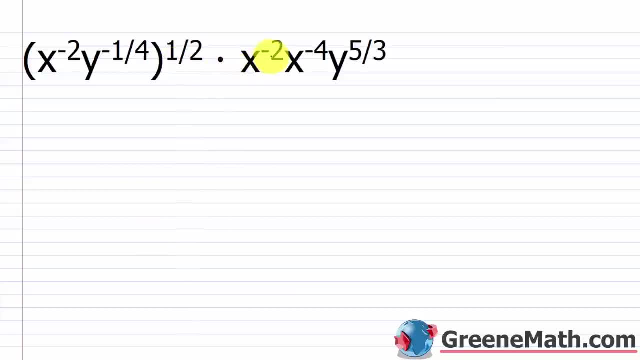 This is raised to the 1 half power. Then we're multiplying by x to the power of negative 2 times x to the power of negative 4 times y to the 5 thirds power. So the first thing I want to do is use my power rule here. So x stays the same in this scenario. And we have negative 2 raised to the 1 half power. So negative 2 times 1 half. We know that this cancels with this. I'd have negative 1. So this is x to the power of negative 1. 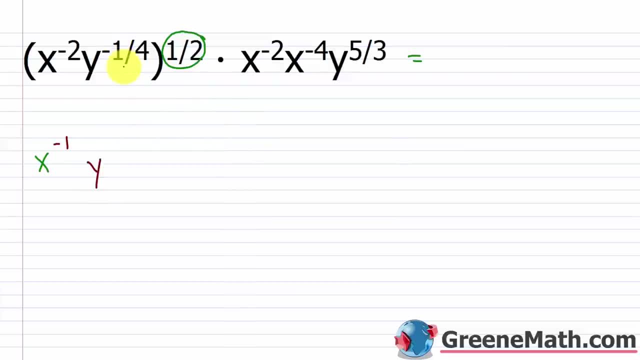 Y, I have the power of negative 1 fourth times 1 half. So 4 times 2 is 8. So this would be negative 1 eighth. Okay, then times. Over here, if I have x and I have x, that stays the same. And then negative 2 plus negative 4 is negative 6. And then lastly, I just have y to the 5 thirds power. So if I have x to the power of negative 1 plus negative 6, which is negative 7. And then as far as y goes, I can combine these. So I'd have y to the power of, if I have negative 1 eighth plus 5 thirds, 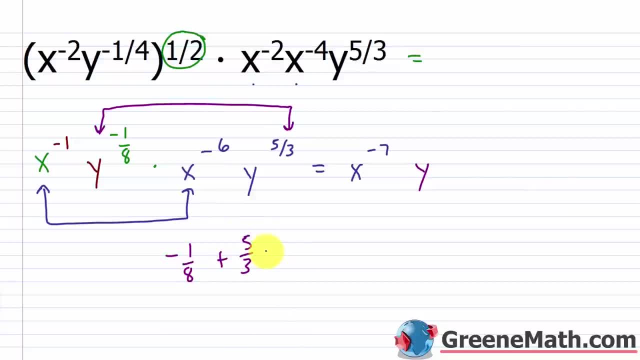 what's that going to be equal to? Well, we've got to have a constant. So we're going to have a common denominator. So let me multiply this by 8 over 8. Let me multiply this by 3 over 3. I would get negative 3 over 24 plus 40 over 24. So this is 37 over 24. 37 over 24. 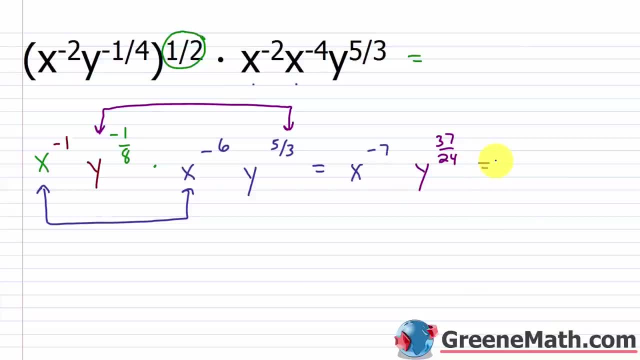 So you can leave it like this, or you could write it as y to the power of 37 over 24. So you can leave it like this, or you could write it as y to the power of 7 over x to the power of 7. 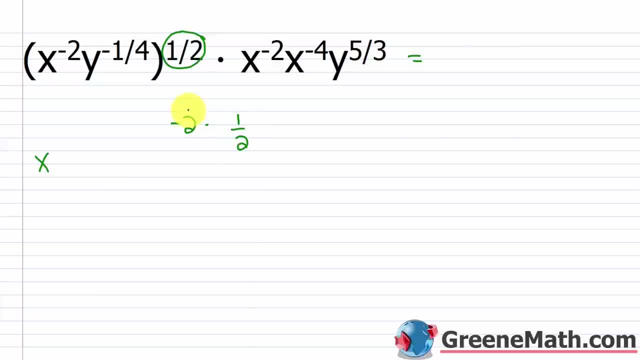 So negative 2 times 1 half. We know that this cancels. with this, I'd have negative 1.. So this is x to the power of negative 1.. And then for y, I have the power of negative 1. fourth, 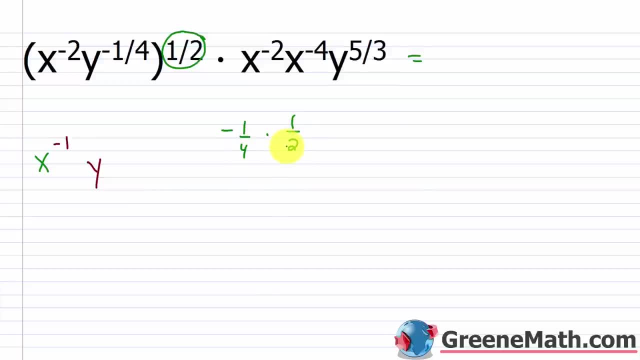 times 1 half. So 4 times 2 is 8, so this would be negative 1. eighth. Okay, then times over here: if I have x and I have x, that stays the same, And then negative 2 plus negative 4 is negative 6.. 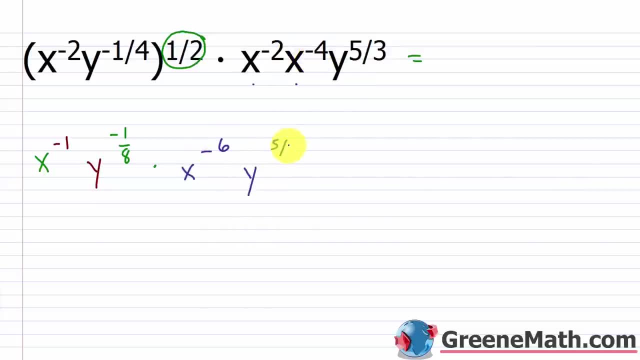 And then, lastly, I just have y to the 5 thirds power. So if I think about these two here, I can combine them using the product rule for exponents. I would have x to the power of negative 1 plus negative 6,. 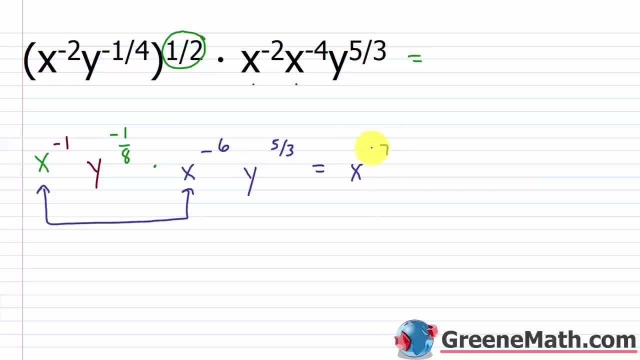 which is negative 7.. And then, as far as y goes, I can combine these, So I'd have y to the power of. if I have negative 1 eighth plus 5 thirds, what's that going to be equal to? 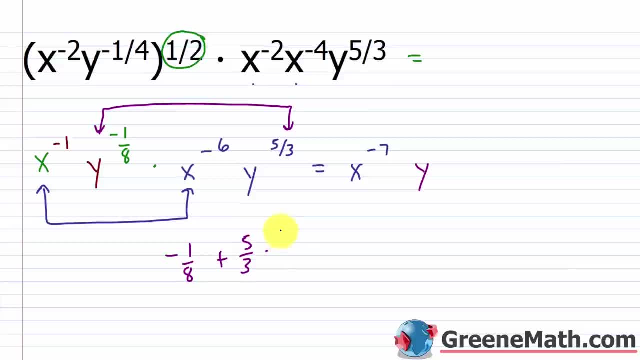 Well, we've got to have a common denominator. So let me multiply this by 8 over 8.. Let me multiply this by 3 over 3.. I would get negative 3 over 24, plus 40 over 24.. 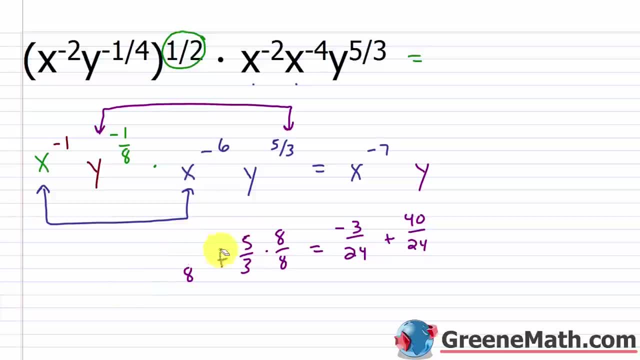 So this is 37 over 24.. 37 over 24.. So you can leave it like this, or you could write it as: y to the power of 37 over 24 over x to the power of 7.. Remember, you can drag this into the denominator. 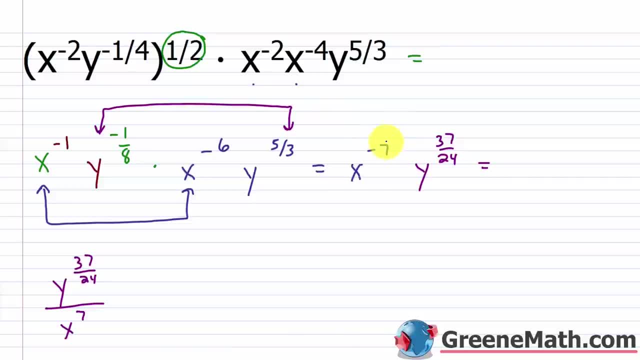 and change the sign of the exponent. So if there's a negative 7, when it's in the numerator, when it gets dragged below into the denominator it becomes positive. Hello and welcome to Algebra 1, Lesson 60.. In this video, 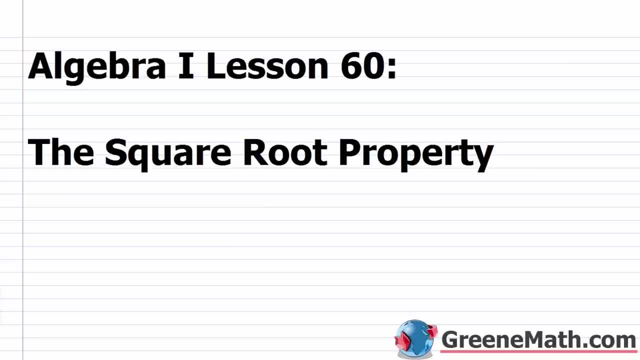 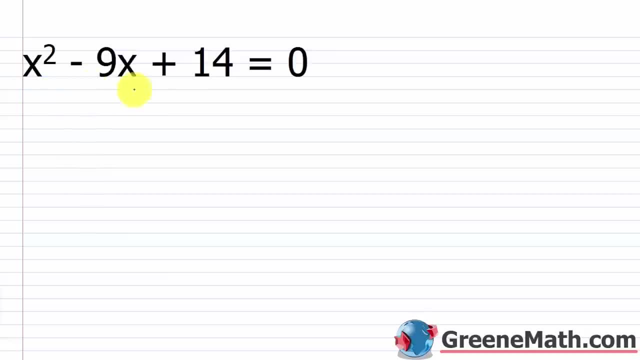 we're going to learn about the square root property. So many lessons ago, we gave you a basic definition for a quadratic equation, So here's an example of one. We have: x squared minus 9x plus 14 equals 0.. So what makes this a quadratic equation? 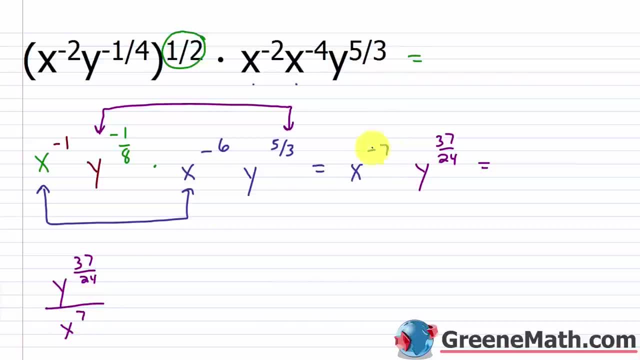 Remember, you can drag this into the denominator and change the sign of the exponent. So if there's a negative 7 when it's in the numerator, when it gets dragged below into the denominator, 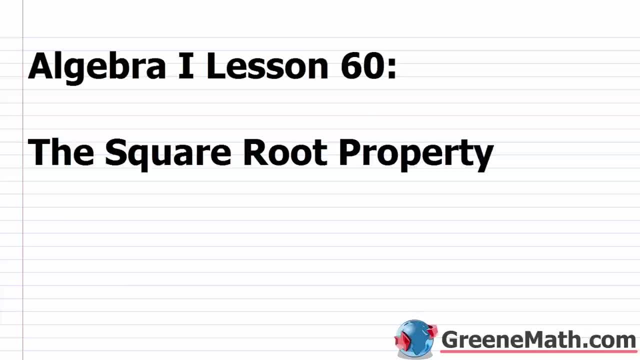 it becomes positive. Hello, and welcome to Algebra 1 Lesson 60. In this video, we're going to learn 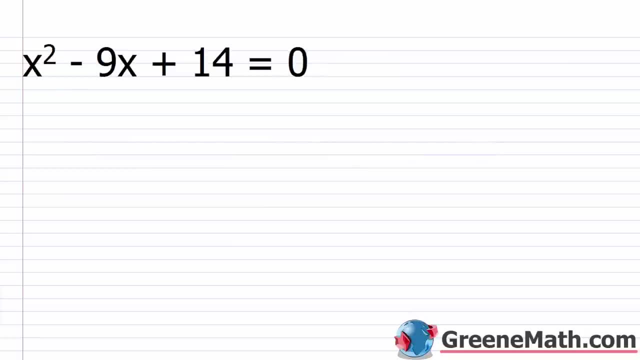 about the square root property. So many lessons ago, we gave you a basic definition for a quadratic equation. So here's an example of one. We have x squared minus 9x plus 14 equals 0. So what makes this a quadratic equation? Well, a quadratic equation has a squared variable, like here we have x squared, and it's got no variable involved with an exponent that's larger than 2. So in other words, if I added x cubed to this, it would no longer be a quadratic equation. Now, another thing this quadratic equation is already in standard form for us. And this is just a convenient way to look at things, and it's displayed such that we have our squared variable all the way to the left, then we have the variable that's to the first power, and then we don't have a variable here. 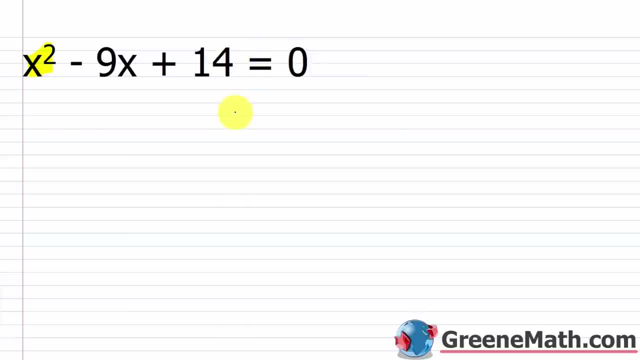 Now, some people in some textbooks will say, well, this is your spot for x to the power of 0. Right, x to the power of 0 is 1. 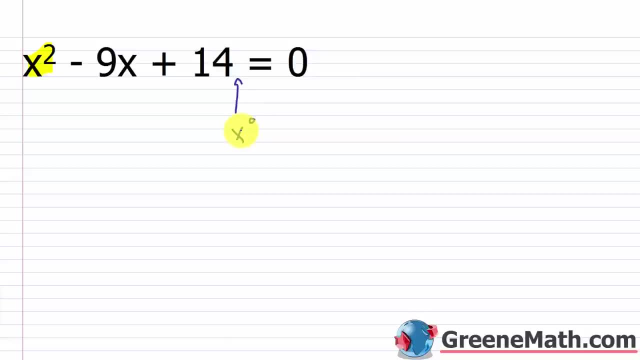 If I multiplied 14 by 1, I just have 14, right? So just kind of a mathy way of looking at that. 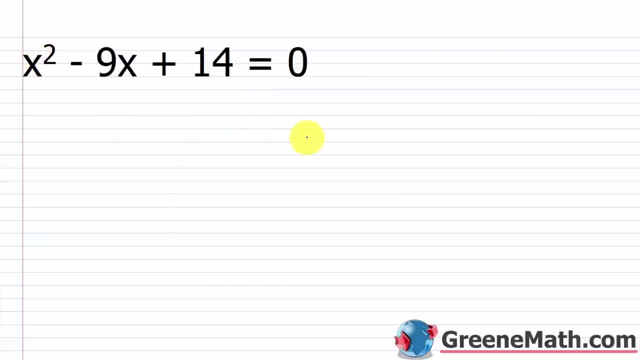 But we've seen quadratic equations before. Up to this point, we've only looked at ones that we could solve by factoring. The purpose of this lesson is to start thinking about techniques that we can use when we can't factor our quadratic equation. So if I have something like x squared 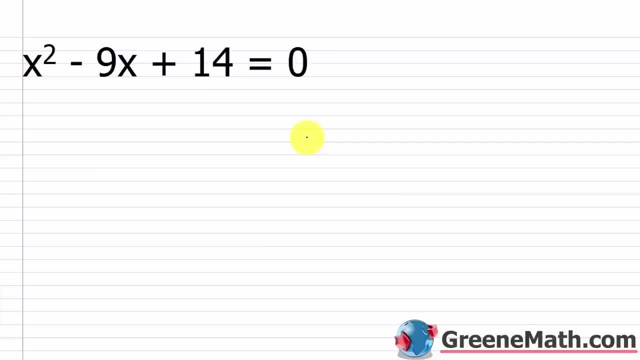 minus 9x plus 14 equals 0, I can actually solve this by factoring. So if I have something like x squared minus 9x plus 14 equals 0, I can actually solve this by factoring. So if I have something like x squared minus 9x plus 14 equals 0, I can actually solve this by factoring. And we're going to do so to get a little bit of a review. 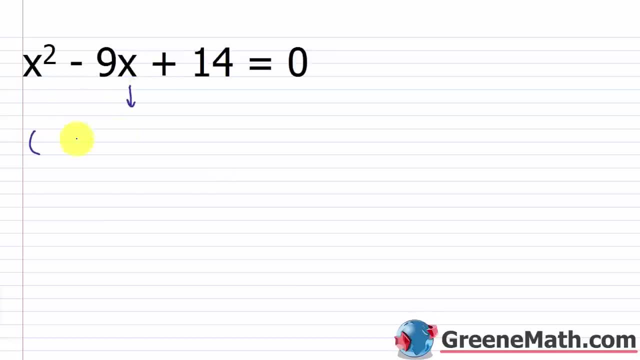 So if I factor the left side here, just like factoring a trinomial, so what would I need? 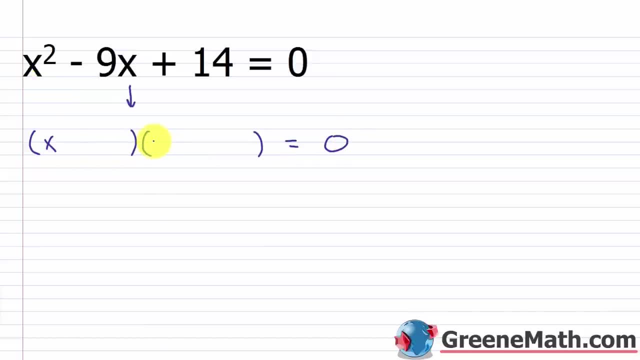 The first position is going to be x, and then the first position here is going to be x as well. And then I want two integers whose sum, 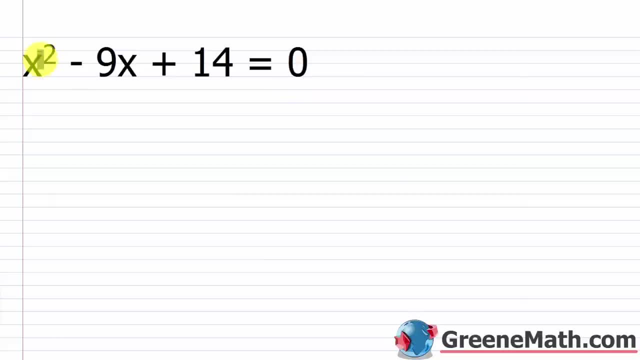 Well, a quadratic equation has a squared variable, like here: we have x squared and it's got no variable involved with an exponent that's larger than 2.. So, in other words, if I added x cubed to this, it would no longer be a quadratic equation. 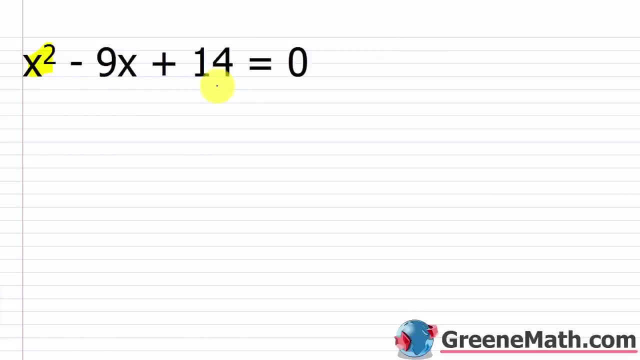 Now, another thing is that this quadratic equation is already in standard form for us- And this is just a convenient way to look at things- and it's displayed such that we have our squared variable all the way to the left. then we have the variable. 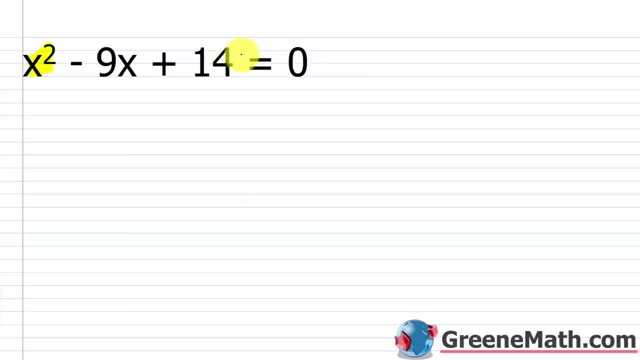 that's to the first power, and then we don't have a variable here. Now some people in some textbooks will say: well, this is your spot for x to the power of 0.. Right x to the power of 0 is 1.. 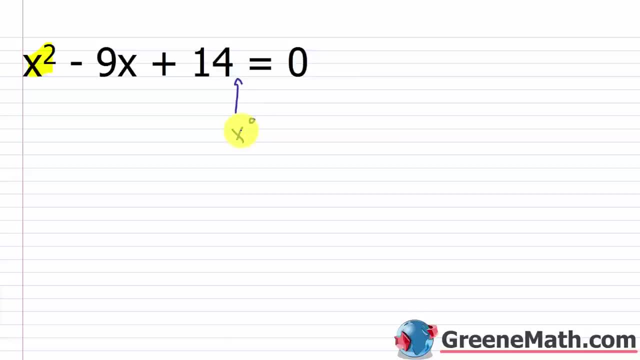 If I multiply 14 by 1, I just have 14.. Right, so just kind of a mathy way of looking at that. But we've seen quadratic equations before. Up to this point we've only looked at ones that we could solve by factoring. 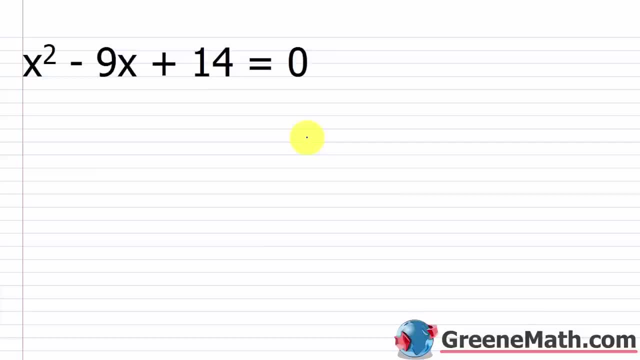 The purpose of this lesson is to start thinking about techniques that we can use when we can't factor our quadratic equation. So if I have something like x squared minus 9x plus 14 equals 0, I can actually solve this by factoring. 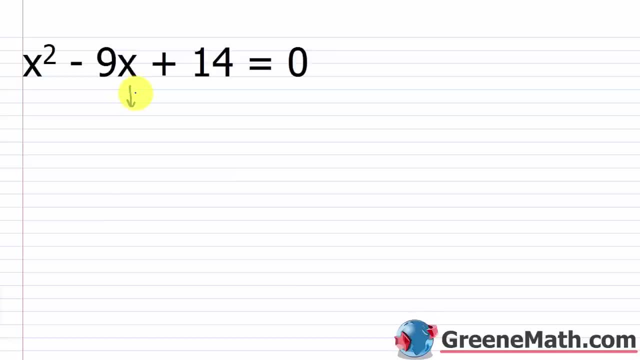 and we're going to do so to get a little bit of a review. So if I factor the left side here, just like factoring a trinomial, so what would I need? The first position is going to be x, and then the first position here: 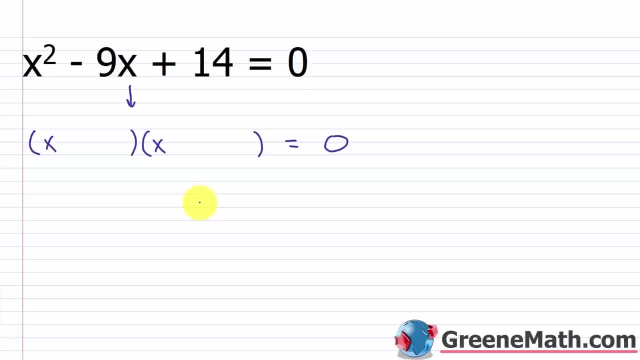 is going to be x as well. And then I want two integers: whose sum? whose sum is negative, 9, and whose product? okay, whose product is 14.. Well, again we think about the factors of 14.. You've got 1 and 14.. 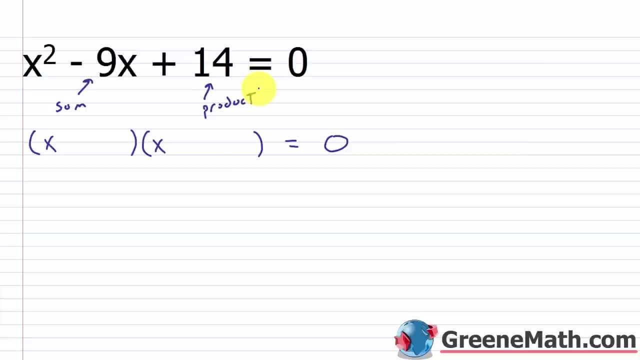 That's not going to work. And then you've got 2 and 7.. If I play with the signs, I can make that work. Notice that you have a negative here and a positive here. Negative plus negative would give me a negative. 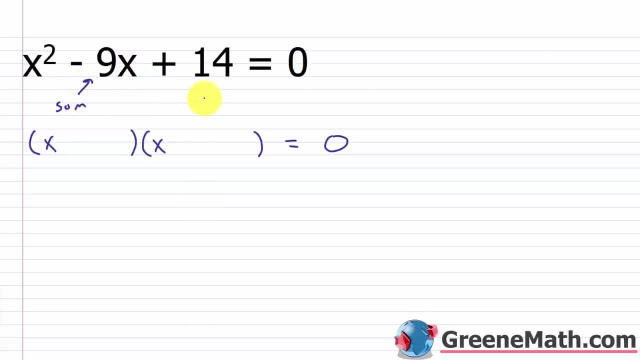 whose sum is negative 9, and whose product, okay, whose product is 14. Well, again, we think about the factors of 14. You've got 1 and 14. That's not going to work. And then you've got 2 and 7. If I play with the signs, I can make that work. Notice that you have a negative here and a positive here. 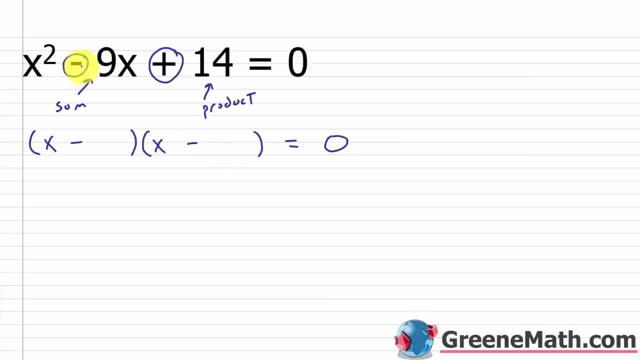 Negative plus negative would give me a negative, and negative times negative would give me a positive. 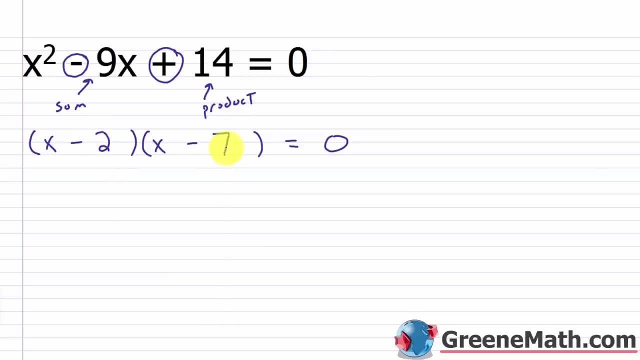 So I want a negative 2 and a negative 7. 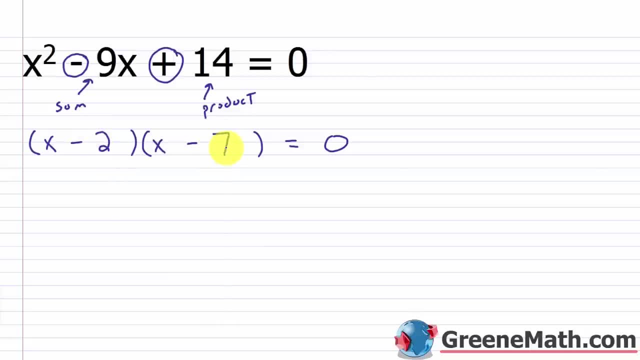 So now that I've factored this into the quantity x minus 2 times the quantity x minus 7, and set this equal to 0, what do I do next? 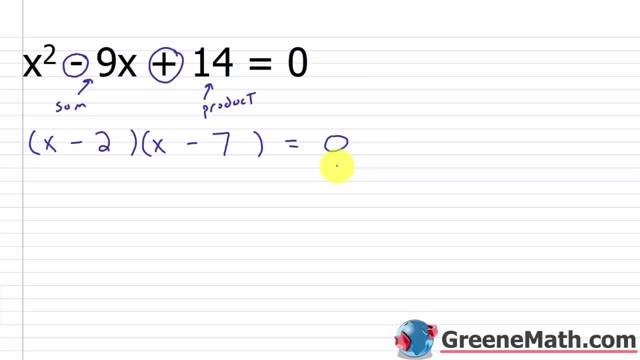 Again, remember I use my zero product property, or some of you call it the zero factor property, doesn't matter. So if I have something like a times b is equal to 0, remember that at least one of these has to be equal to 0 for this to be true. a could be equal to 0, b could be equal to 0, or they both could be equal to 0. Well, following the same logic here, remember these are each factor, that's multiplication, so this is a factor, and then this is a factor. 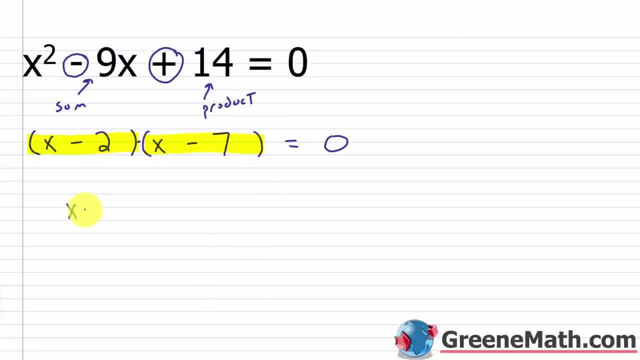 So just like I did there, I would say that either x minus 2 is equal to 0, or x minus 7 is equal to 0, or they're both equal to 0. 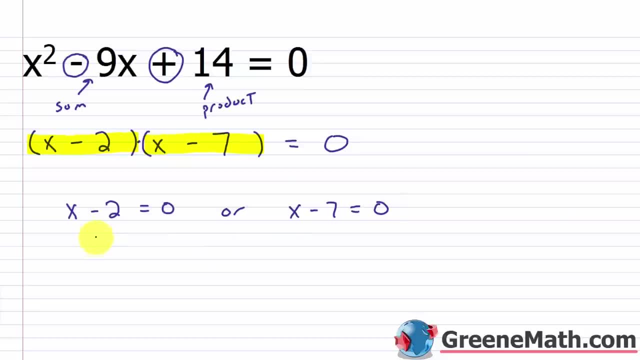 So I would just solve each resulting equation, add 2 to both sides over here, and I'll get x is equal to 2. Then OR, add 7 to both sides of the equation here, I get x is equal to 7. 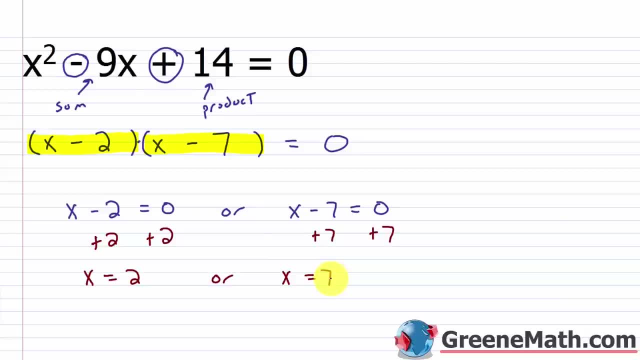 So this equation has two solutions, x could be equal to 2, or x could be equal to 7. 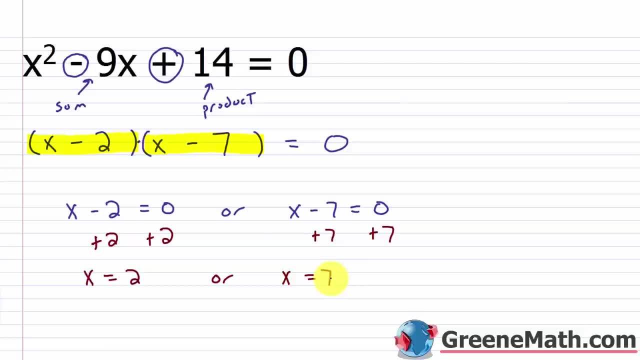 In the interest of time, I'm not going to go through and plug things in and show you that the left and the right side are equal in value. You can pause the video at this point and do that for yourself. I can assure you that both solutions are valid. 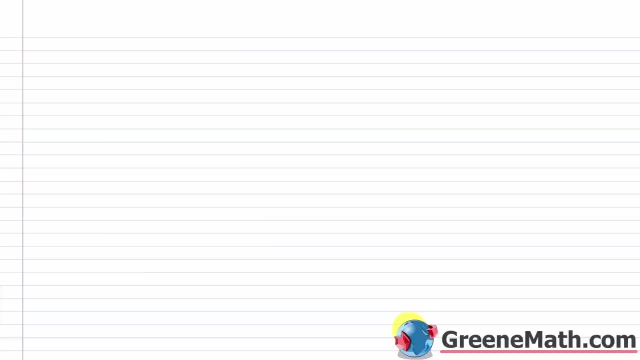 So now that we've reviewed how to solve a quadratic equation by factoring, what happens if we get something that we can't factor? And I'm going to start out with something that we can factor, just so I can prove it to you. 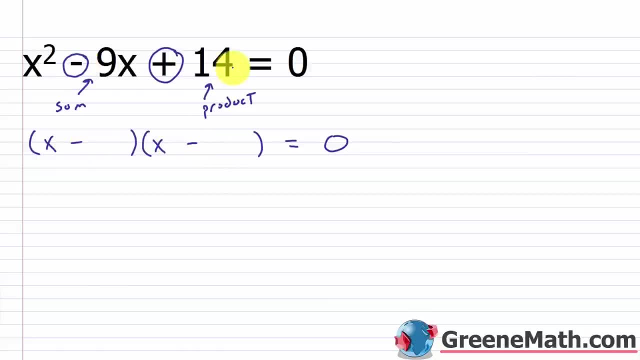 and negative times. negative would give me a positive, So I want a negative 2 and a negative 7.. So now that I've factored this into the quantity x minus 2 times the quantity x minus 7 and set this equal to 0,, 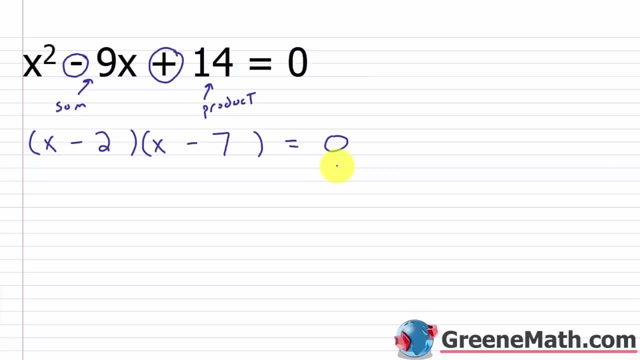 what do I do next? Again, remember I used my zero product property, or some of you call it the zero factor property. It doesn't matter. So if I have something like a times b is equal to 0, remember that at least one of these 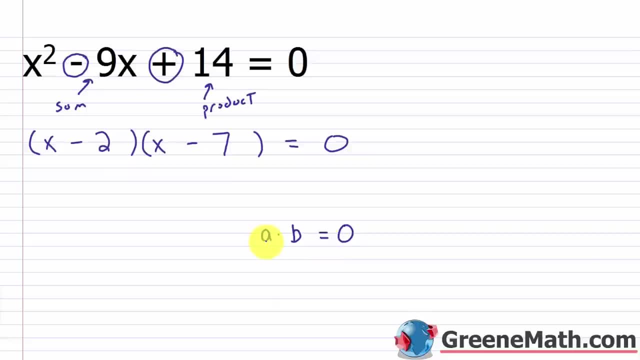 has to be equal to 0 for this to be true. a could be equal to 0,. b could be equal to 0, or they both could be equal to 0.. Well, following the same logic here- remember, these are each factors- 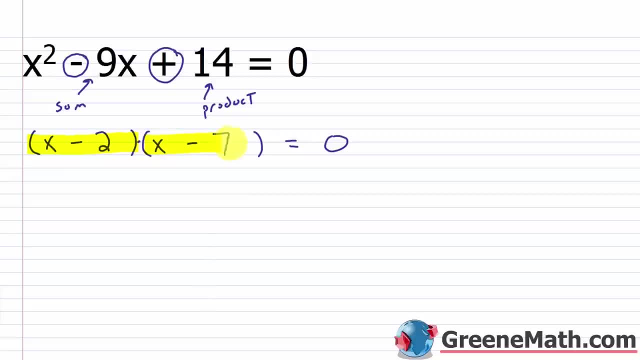 That's multiplication. So this is a factor, and then this is a factor. So, just like I did there, I would say that either x minus 2 is equal to 0, or x minus 7 is equal to 0, or they're both equal to 0.. 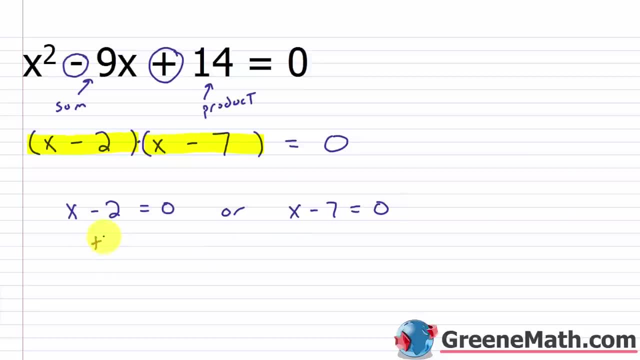 So I would just solve each resulting equation: add 2 to both sides over here, and I'll get x is equal to 2, and or add 7 to both sides of the equation- here I get x is equal to 7.. 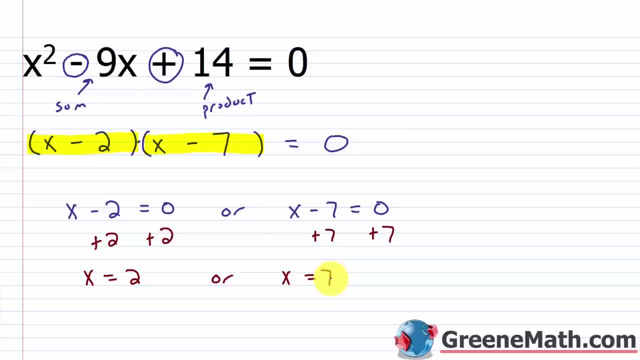 So this equation has two solutions: x could be equal to 2, or x could be equal to 7.. In the interest of time, I'm not going to go through and plug things in and show you that the left and the right side. 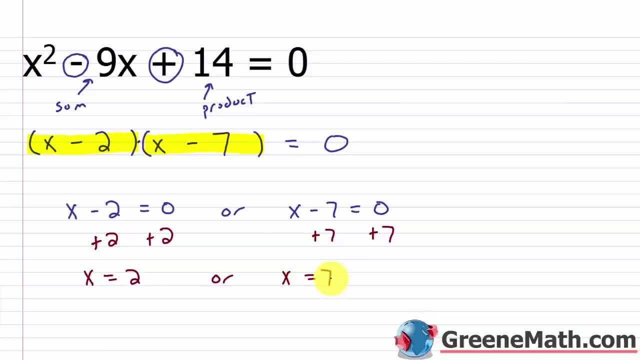 are equal in value. You can pause the video at this point and do that for yourself. I can assure you that both solutions are valid. So, now that we've reviewed how to solve a quadratic equation by factoring, what happens if we get something? 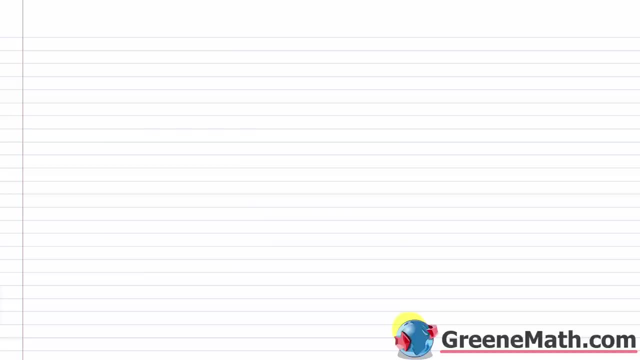 that we can't factor, And I'm going to start out with something that we can factor, just so I can prove it to you. but let's just say, for example: I give you something really, really easy, So we have x squared. 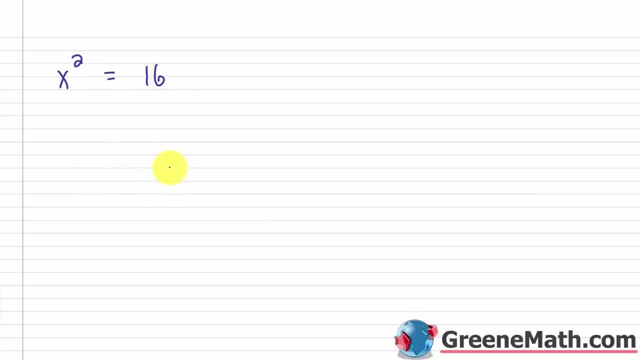 is equal to 16.. Now, this, by definition, is a quadratic equation. I have a squared variable here and I have no variable with any higher value or higher power, And I realize that some of you will say: well, you're missing. 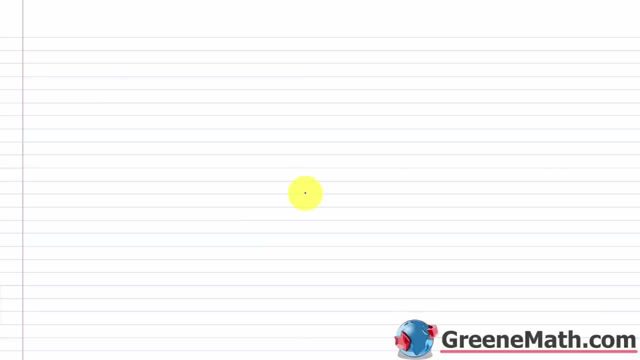 But let's just say, for example, I give you something really, really easy. So we have x squared is equal to 16. Now this, by definition, is a quadratic equation. I have a squared variable here, and I have no variable with any higher power. And I realize that some of you will say, well, you're missing the x to the first power. That doesn't matter, it's still a quadratic equation. So how would I go about solving this for x? I want you to use what you've learned up to this point to think about how I would isolate, how I would isolate x, isolate x. 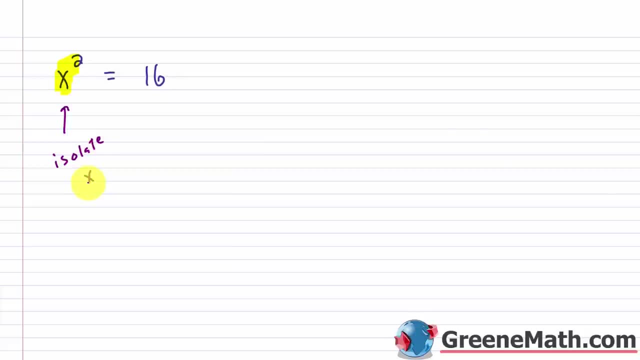 Well, think about when we isolate the variable, we're usually trying to undo what's being done to it. 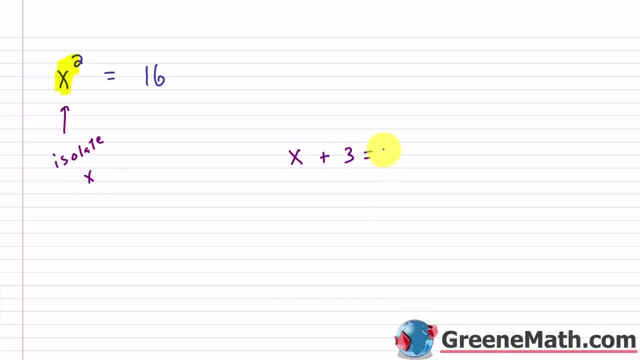 If I have an equation like x plus 3 equals 7, 3 is being added to x, so I do the opposite, and I subtract 3 away from each side, and I get x is equal to 4. 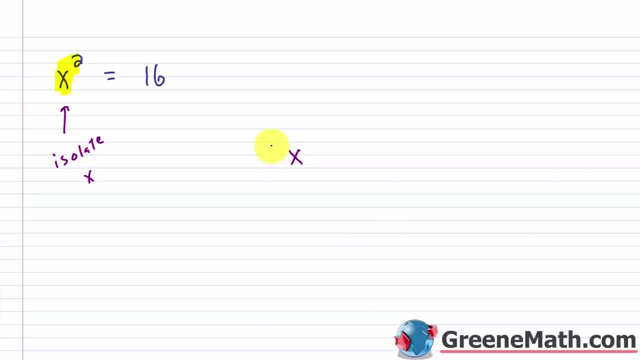 If I have multiplication, something like 6x equals 24, since 6 is multiplying x, I do the opposite, which is division, to both sides of the equation, and this becomes x is equal to 4. 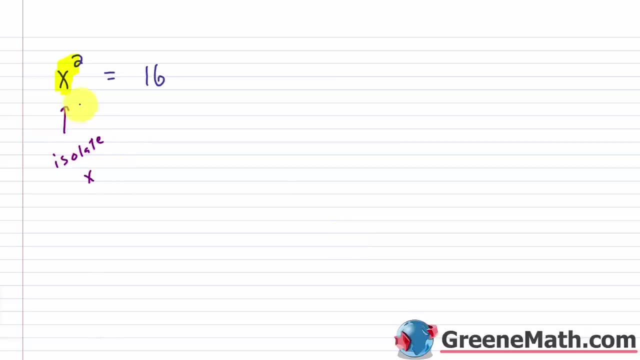 So just like with these basic examples, I want to, again, isolate x, and if I'm squaring x, the opposite of that is to take the square root. 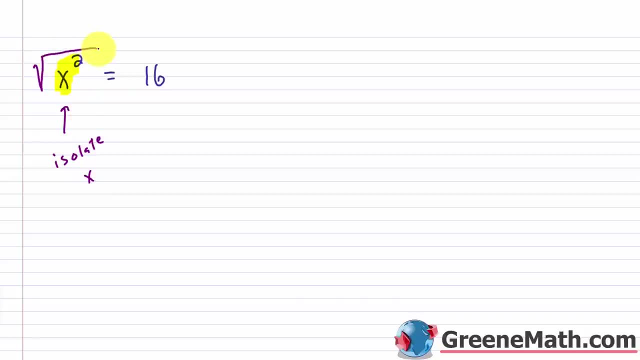 So if I take the square root of this side, what's going to happen is this will cancel with this, and I'll be left with x. 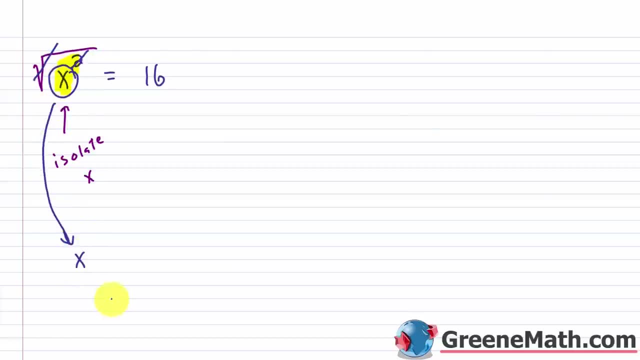 So I have isolated x, I have successfully done that. But again, just like when we use the addition property of equality, and we use the multiplication property of equality, we've got to do the same thing to each side, so I've got to take the square root over here. 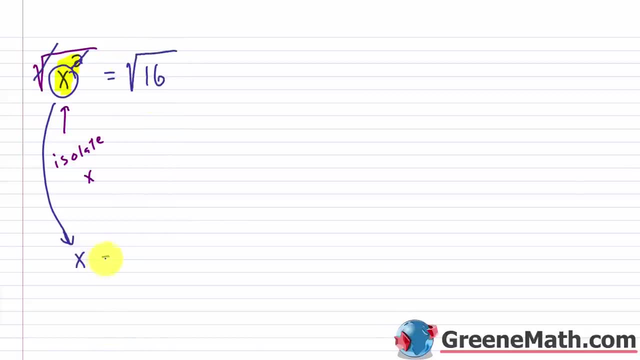 Now the square root of 16 is 4, so let's put x equals 4. 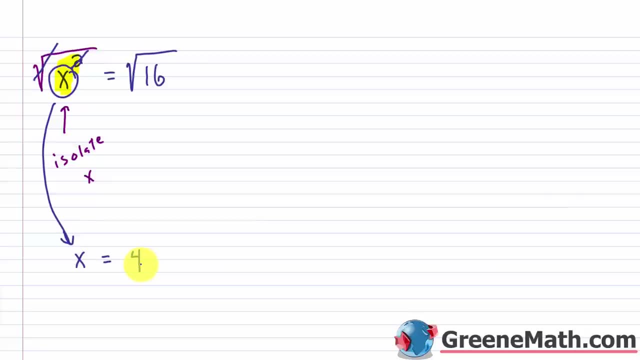 Now are we done? Is this our correct answer? Well, it's partially correct. X does equal 4. 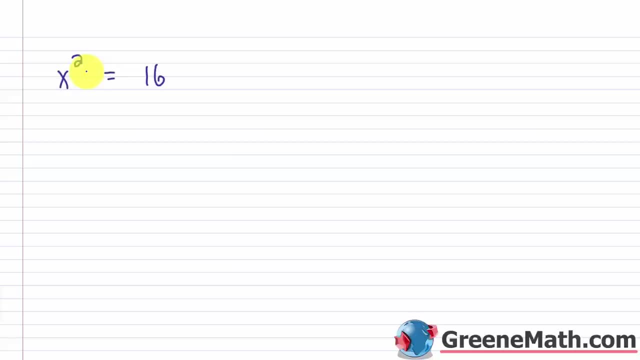 the x to the first power. That doesn't matter. It's still a quadratic equation. So how would I go about solving this for x? I want you to use what you've learned up to this point to think about how I would isolate. 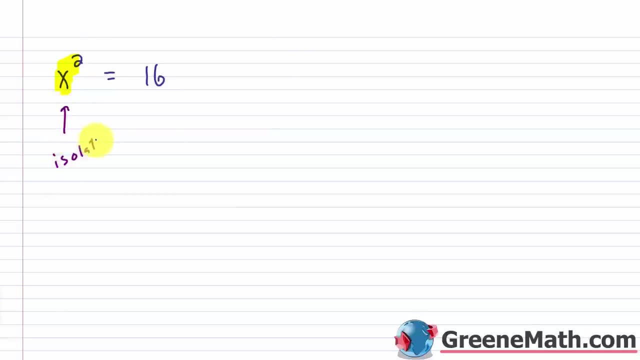 how I would isolate x, Isolate x. Well, think about. when we isolate the variable, we're usually trying to undo what's being done to it. If I have an equation like x plus 3 equals 7, 3 is being added to x. 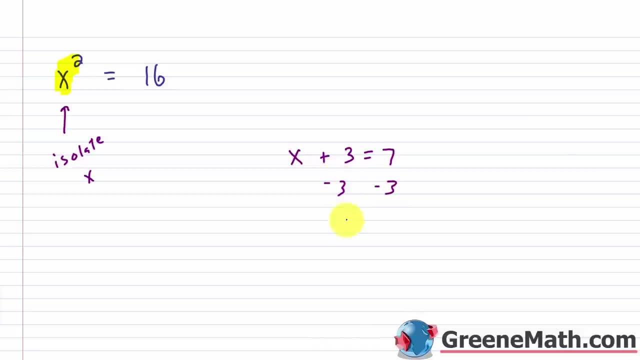 so I do the opposite and I subtract 3 away from each side and I get x is equal to 4.. If I have multiplication, something like 6x equals 24, since 6 is multiplying x, I do the opposite. 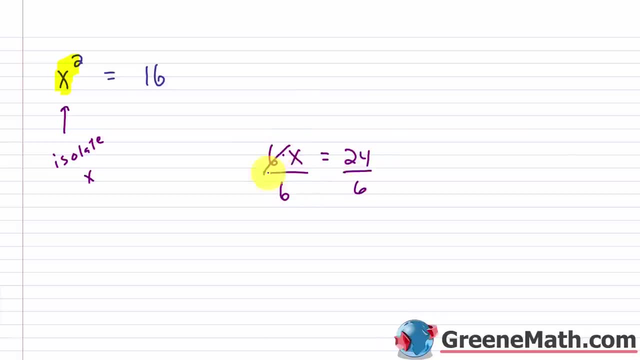 which is division to both sides of the equation, and this becomes: x is equal to 4.. So, just like with these basic examples, I want to again isolate x, and if I'm squaring x, the opposite of that is to take the square root. 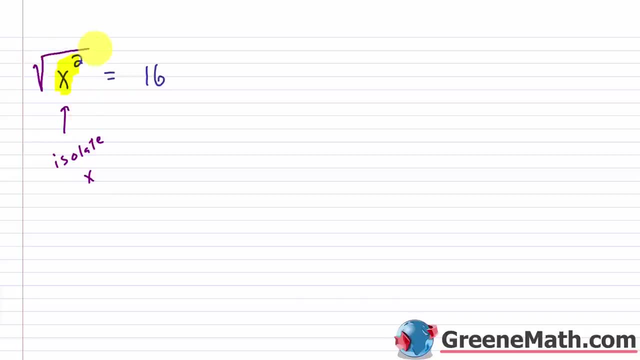 So if I take the square root of this side, what's going to happen is: this will cancel with this and I'll be left with x. So I have isolated x. I have successfully done that, But again, just like when we use the addition. 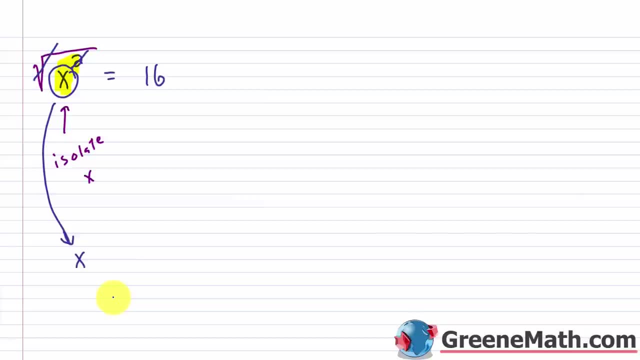 property of equality and we use the multiplication property of equality. we've got to do the same thing to each side, So I've got to take the square root over here. Now. the square root of 16 is 4.. So let's put: x equals 4.. 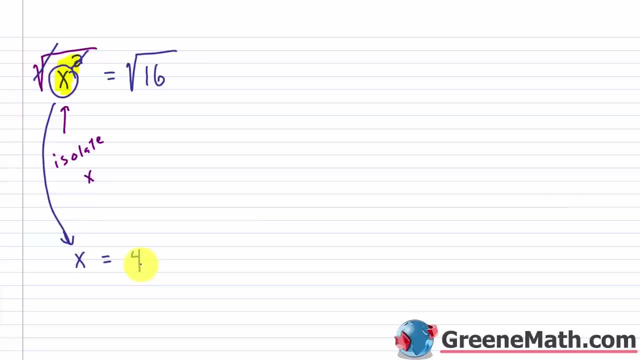 Now are we done. Is this our correct answer? Well, it's partially correct. x does equal 4.. But x here can also be equal to negative 4.. And let me show you why. we miss this when we first start doing it. 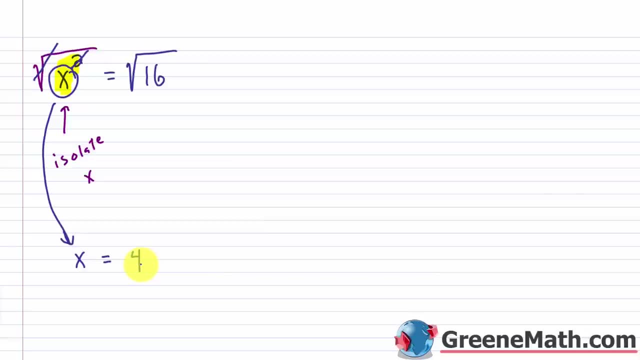 But x here can also be equal to negative 4. And let me show you why we miss this when we first start doing it. Recall a few lessons ago that we defined this symbol right here to mean the principal square root. 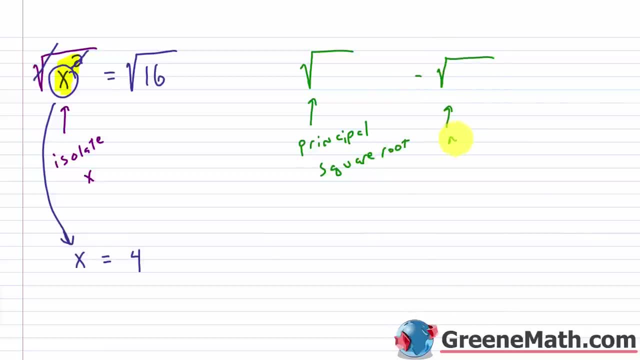 And we defined this symbol to be the negative, the negative square root. 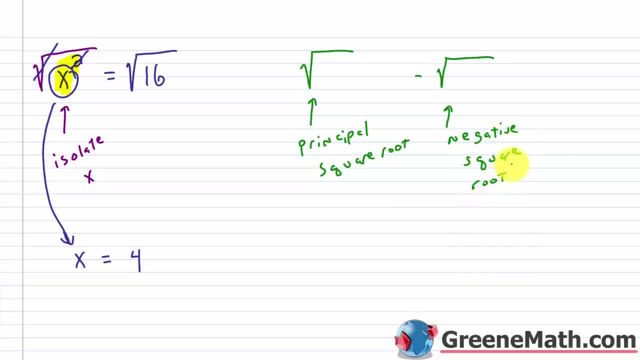 And why did we show two different things? Well, it's kind of a notational thing. Now when we first started talking about square roots, if I said, what is the square root 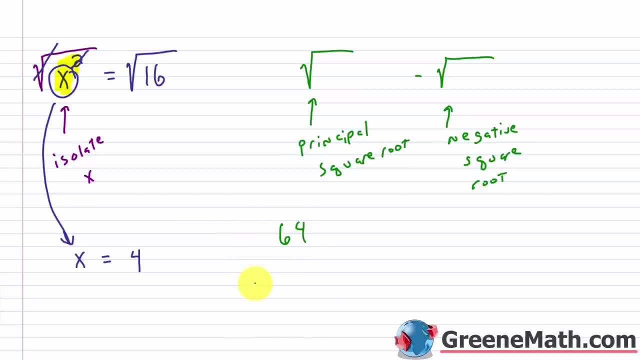 of 64, I'm not even going to put the symbol, I first defined it by saying, give me a number that when multiplied by itself would give you 64. 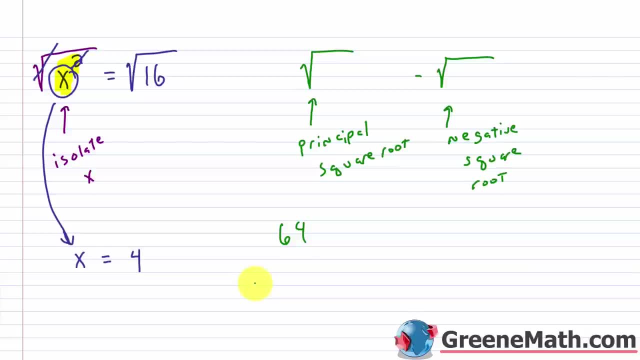 Well, you know that eight would do that, but also negative eight would do that. So to account for the two possibilities. 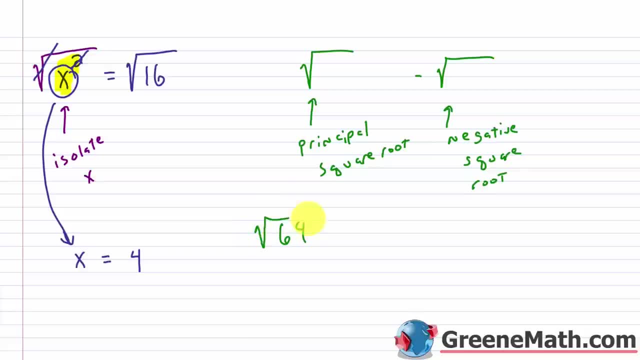 If I wanted the principal or positive square root of 64, I would do that. And if I wanted the negative square root of 64, I would do that. So this would produce negative 8. 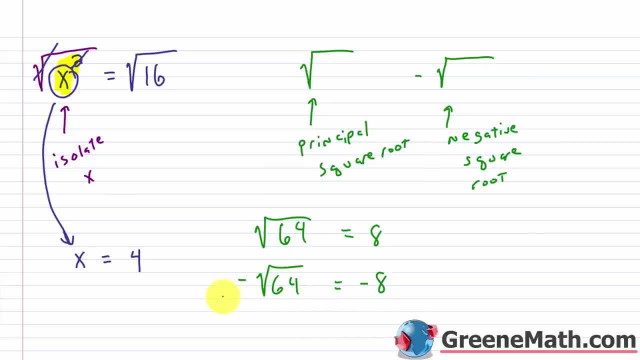 Now, what we didn't do here is account for the fact that negative 4 squared would also give us 16. So what's going to happen is when we take the square root of both sides, let me kind of clean this up and go back to what we had originally. When we take the square root of each side, we've got to put a symbol out in front over here that says plus or minus. 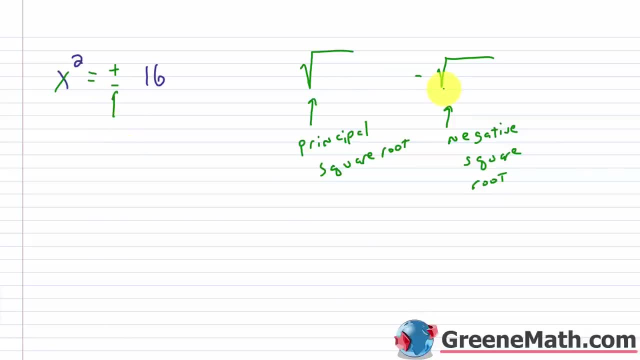 And this is just notation that refers to these two different scenarios. 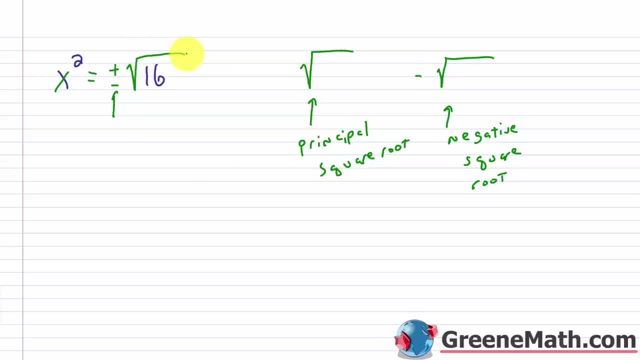 I want to take the positive and the negative square root of 16 when I do this. So this will cancel with this, and I have x equals plus or minus square root of 16 is 4. So this is actually... This is actually two different solutions. 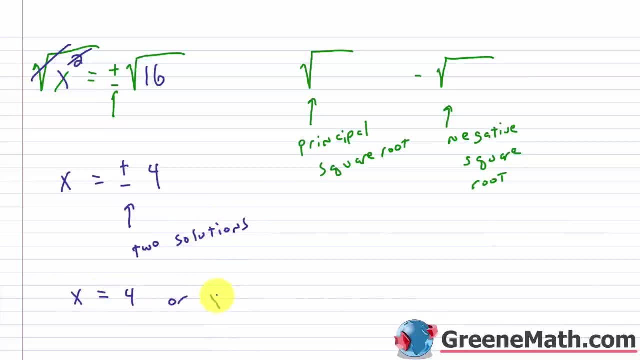 This is x is equal to 4 or x is equal to negative 4. And there's a lot of ways to prove that to yourself. If you just go back to the original equation, if I plug in a 4, 4 squared is 16. 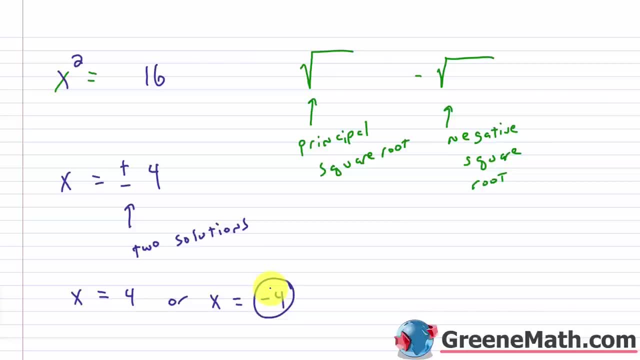 If I plug in a negative 4 where the negative and the 4 are inside of parentheses, I square that, I would also get 16. 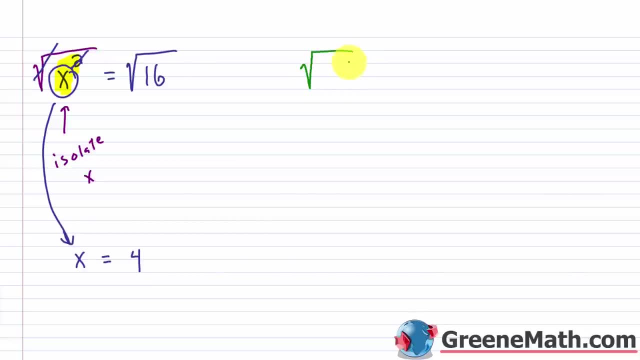 Recall a few lessons ago that we defined this symbol right here to mean the principal square root, And we defined this symbol to be the negative, the negative square root. And why did we show two different things? Well, it's kind of a notational thing. 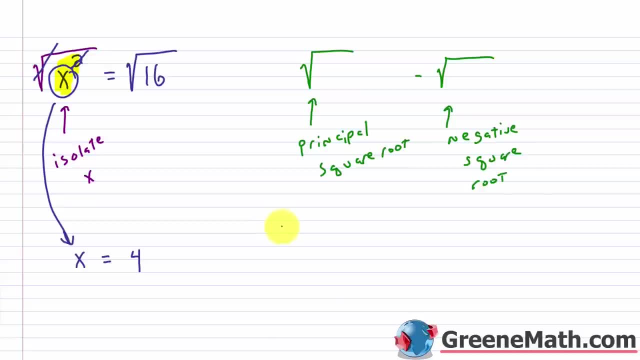 Now, when we first started talking about square roots, if I said what is the square root of 64, what's the symbol, I first defined it by saying: give me a number that, when multiplied by itself, would give you 64.. Well, you know that. 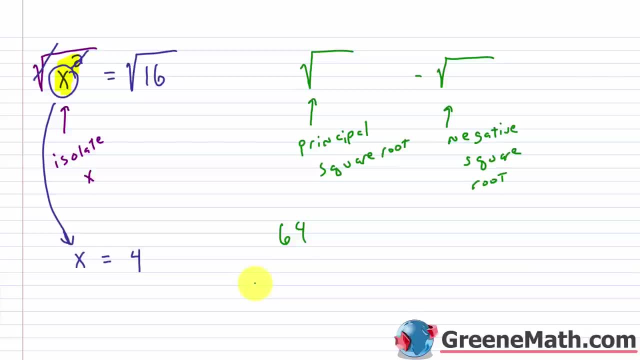 8 would do that, but also negative 8 would do that. So to account for the two possibilities, if I wanted the principal or positive square root of 64, I would do that, And if I wanted the negative square root of 64,, 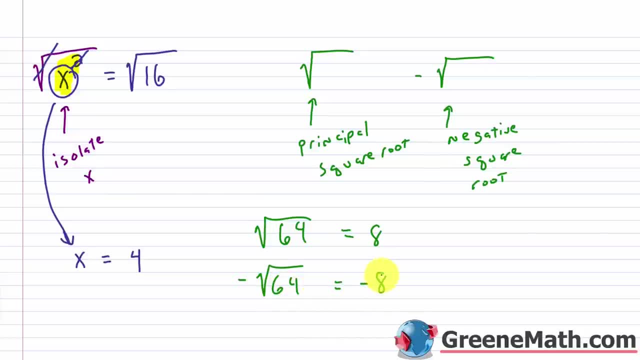 I would do that. So this would produce negative 8.. Now what we didn't do here is account for the fact that negative 4 squared would also give us 16. So what's going to happen is when we take the square root. 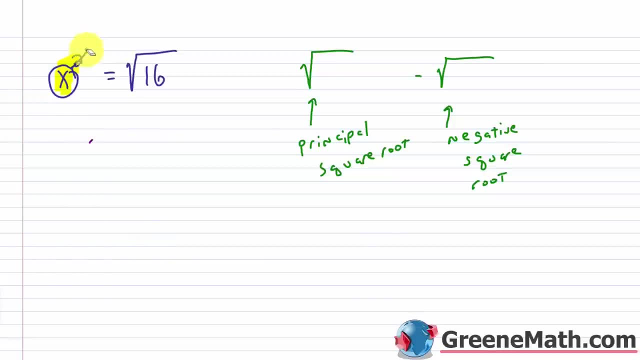 of both sides. let me kind of clean this up and go back to what we had originally. When we take the square root of each side, we've got to put a symbol out in front over here that says plus or minus, And this is just notation. 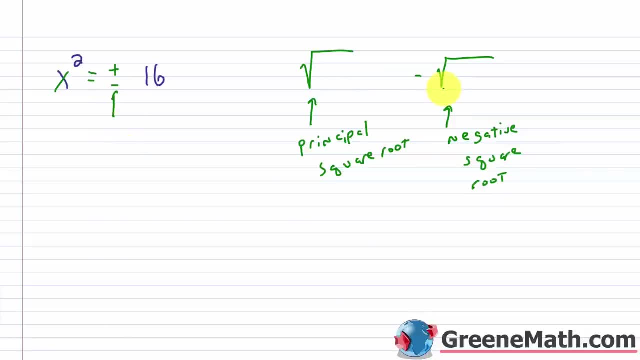 that refers to these two different scenarios. I want to take the positive and the negative square root of 16 when I do this, So this will cancel with this, and I have x equals plus or minus. square root of 16 is 4.. 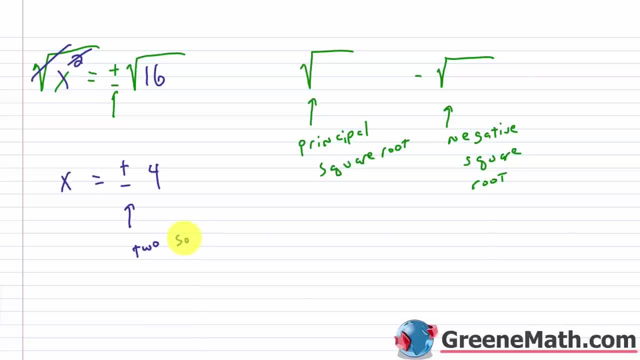 So this is actually two different solutions. Two solutions. This is x is equal to 4 or x is equal to negative 4.. And there's a lot of ways to prove that to yourself If you just go back to the original equation. 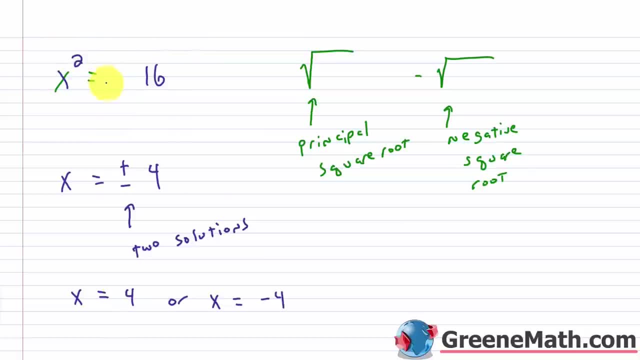 if I plug in a 4,, 4 squared is 16.. If I plug in a negative 4 where the negative and the 4 are inside of parentheses, I square that. I would also get 16.. And one last quick way. 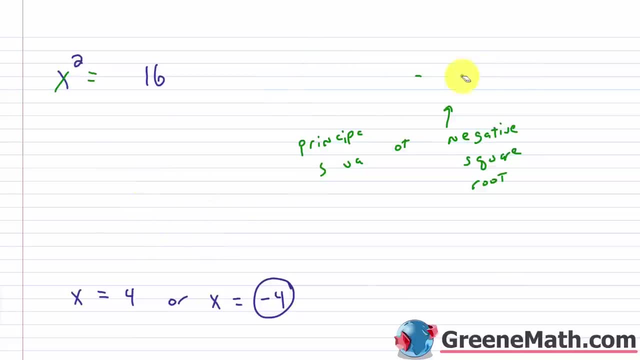 And one last quick way to prove that to you, just use what you know. 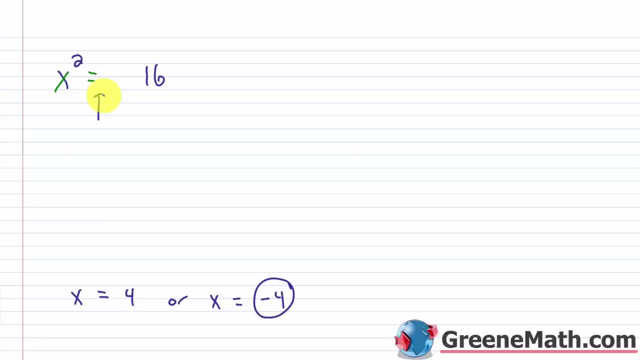 Let's say that I looked at this equation in a different way. Let's say that we go over here and we say that, okay, we have x squared is equal to 16. I want you to subtract 16 away from each side of the equation. So we know this would cancel and become 0. Now, can I factor the left side of this equation? Yes, I can. 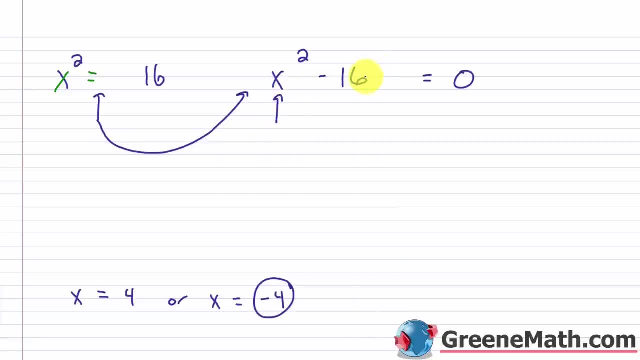 This is the difference of two squares. I have x squared. And really, I could write 16 if I wanted to as 4 squared. 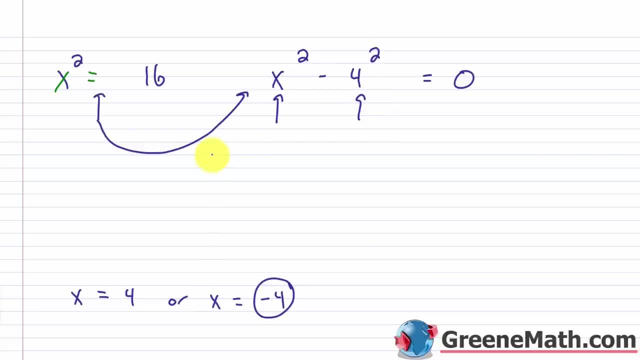 Okay, so the difference of two squares, which factors into x plus 4, that quantity, times x minus 4, that quantity, and this equals 0. 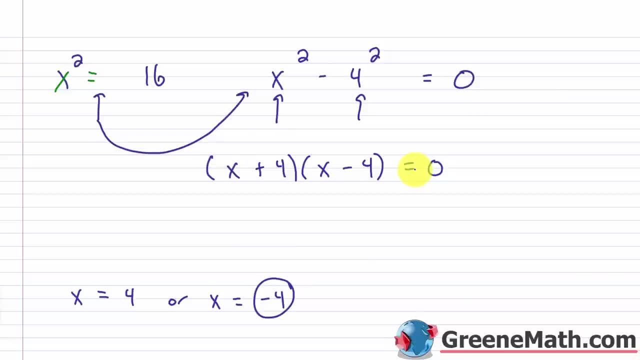 If I set each of these factors equal to 0 and I solve, we know that we have x plus 4 equals 0 or x minus 4 equals 0, which gives us... two solutions. 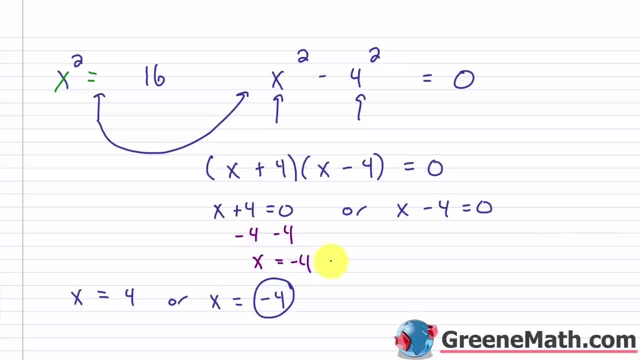 This one, subtract 4 away from each side, you get x equals negative 4. 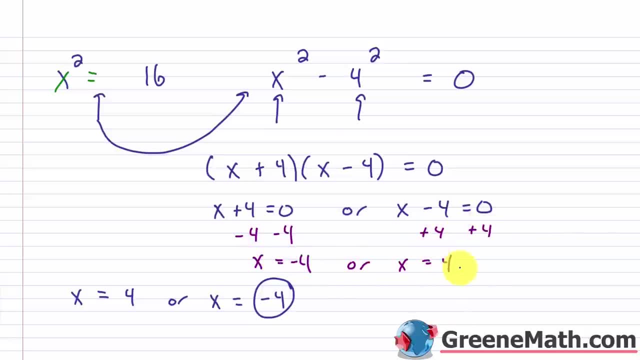 This one, add 4 to both sides, and you get x is equal to 4. So that's exactly what we got here. 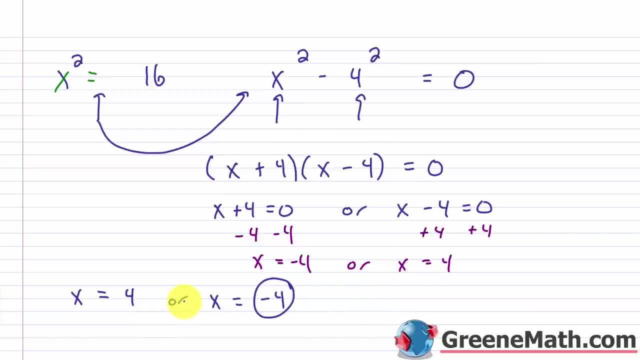 So you can see that using this square root property, which I'm going to define for you in a minute, gives you the same answer as when you solve it using factoring. 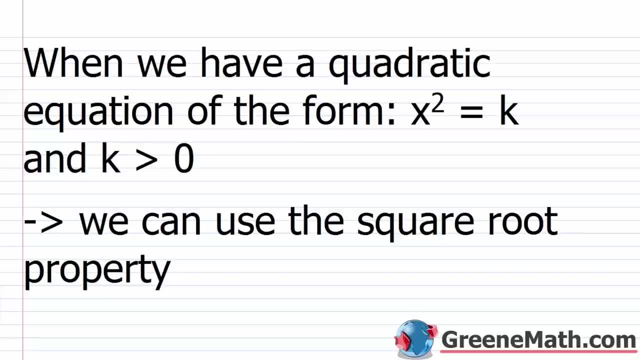 All right, so let's go over the official definition of the square root property. So when we have a quadratic equation of the form, x squared equals k. 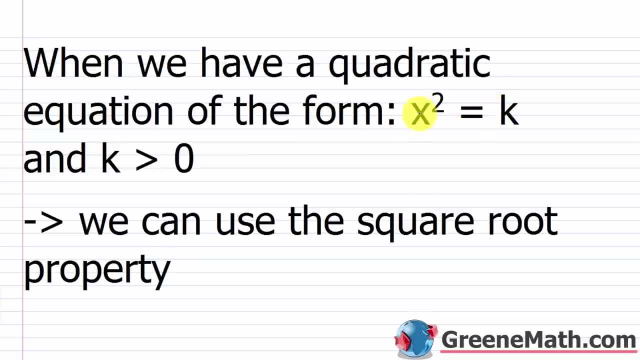 So something squared, it doesn't have to absolutely be x. We'll see some more complicated examples at the end of this lesson, but let's just take this slow. So let's just say we have x squared is equal to some number k. And k is greater than 0, so that means k is positive. Well, then we can use the square root property to get a solution. And the square root property looks like this. 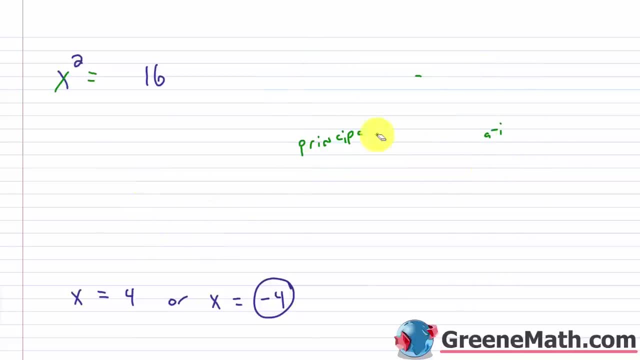 to prove that to yourself, just use what you know. Let's say that I looked at this equation in a different way. Let's say that we go over here and we say that, okay, we have x, squared is equal to 16.. 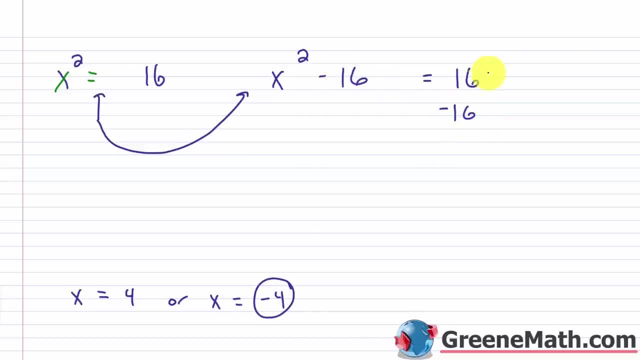 I want you to subtract 16 away from each side of the equation. So we know this would cancel and become zero. Now can I factor the left side of this equation? Yes, I can. This is the difference of two squares. I have x squared. 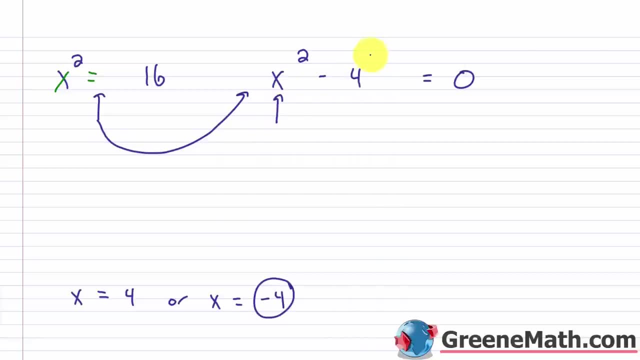 and really I could write 16 if I wanted to, as 4 squared. Okay, so the difference of two squares, which factors into x plus 4, that quantity times x minus 4, that quantity and this equals 0.. 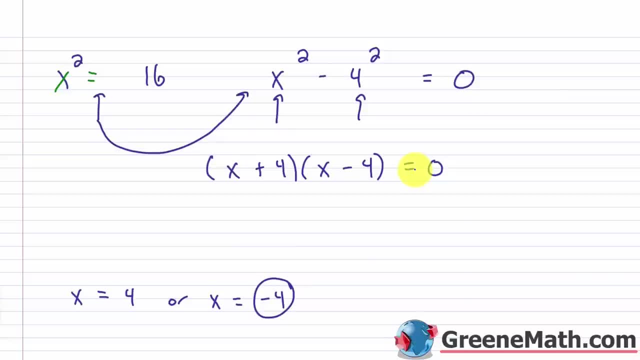 If I set each of these factors equal to 0 and I solve, we know that we have x plus 4 equals 0, or x minus 4 equals 0,, which gives us two solutions. This one subtract 4 away from each side. 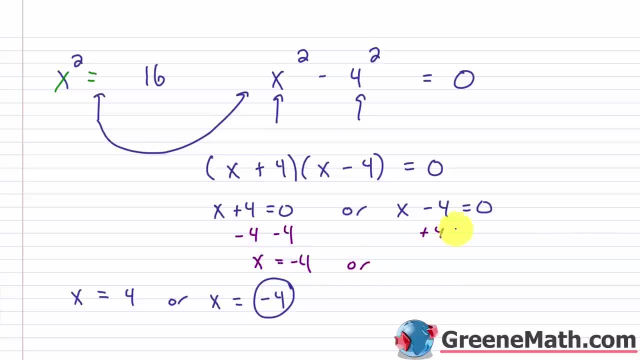 you get x equals negative 4.. This one, add 4 to both sides and you get x is equal to 4.. So that's exactly what we got here, So you can see that when you're using this square root property. 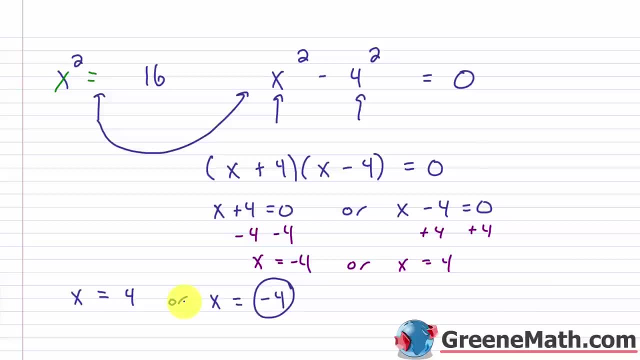 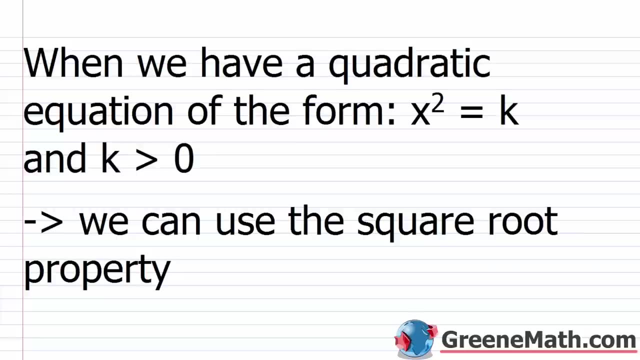 which I'm going to define for you in a minute, gives you the same answer as when you solve it using factoring. All right, so let's go over the official definition of the square root property. So when we have a quadratic equation of the form, 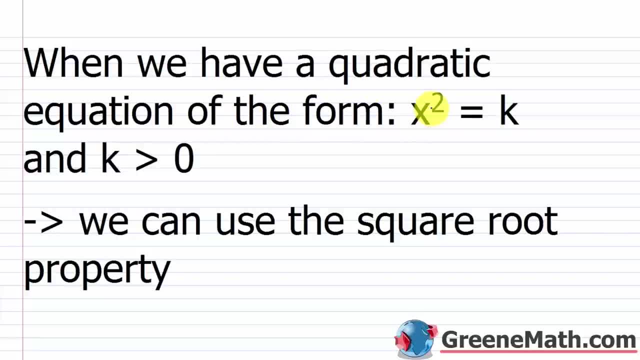 x squared equals k. So something squared, it doesn't have to absolutely be x. We'll see some more complicated examples at the end of this lesson, but let's just take this slow. So let's just say we have x squared is equal to. 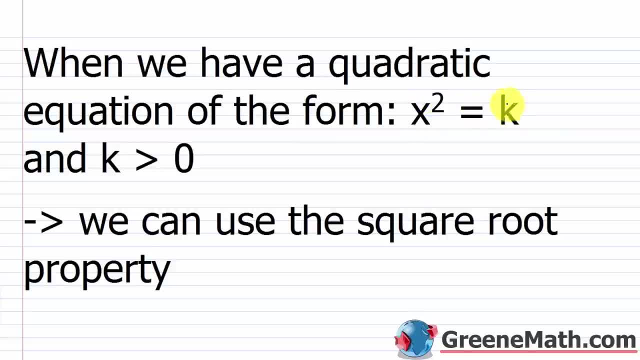 some number- x squared, x squared, x squared- some number- k and k is greater than 0. So that means k is positive. Well then, we can use the square root property to get a solution. And the square root property. 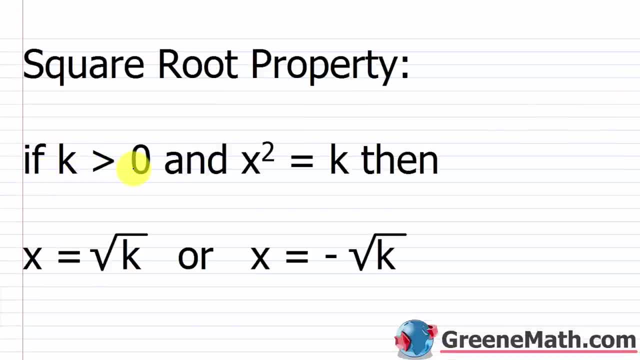 looks like this Again: if k is greater than 0, meaning k is positive and x squared is equal to k, then x is equal to the principal square root of k. so the principal, or x, is equal to the negative. 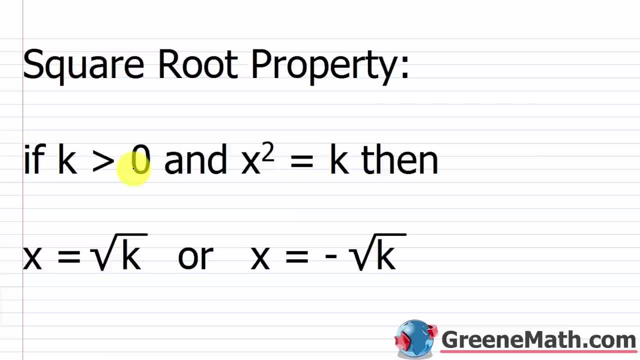 Again, if k is greater than 0, meaning k is positive, and x squared is equal to k, then x is equal to the principal square root of k, so the principal, or x is equal to the negative, the negative square root of k. 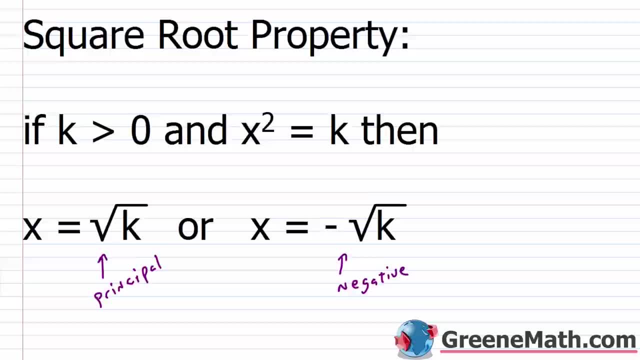 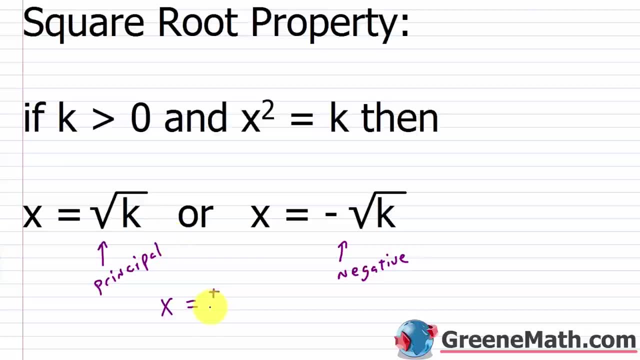 And generally what we do to save space is we'll write x is equal to the positive or principal square root of k, and then we put the negative underneath, and then we write square root of k. So x equals plus or minus, that's how it's read, plus or minus the square root of k. This is just a compact way to write this. 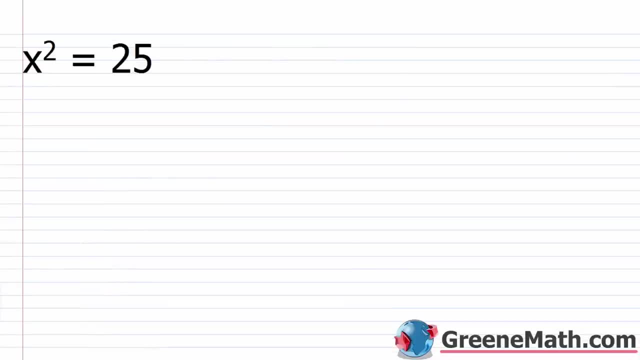 Okay, so let's take a look at an easy one. So we have x squared equals 25. 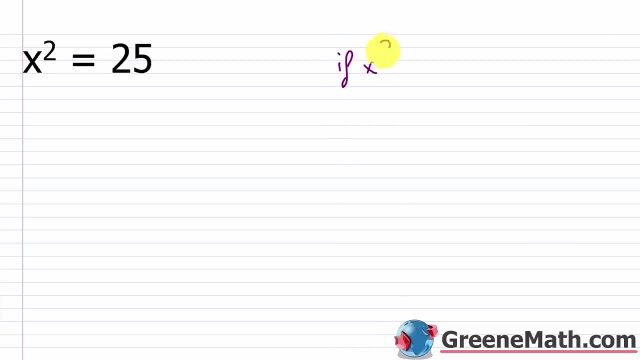 So again, if x squared is equal to k, and k is greater than 0, then x is equal to plus or minus the square root of k. 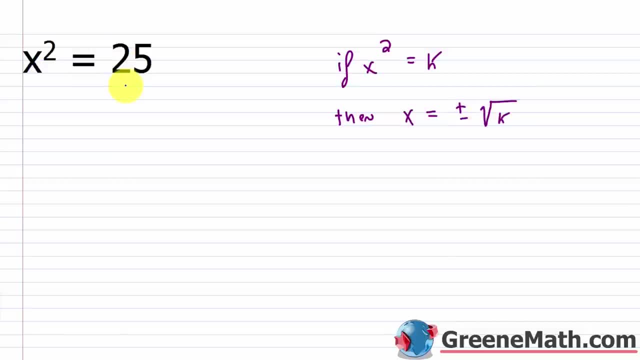 So I'm going to do that over here. I'm going to take the square root of each side, but again, I've got to account for the positive and the negative version. So let's write that down here. So we'll have x squared is equal to 25, and I'm going to take the square root of this side, and then over here I'm going to put plus or minus the square root of this side. 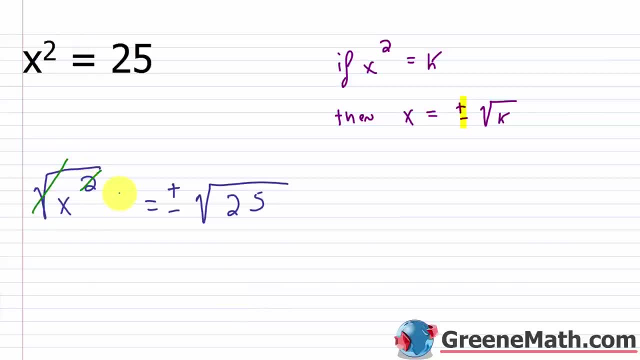 So we know at this point that this cancels with this, and we'll have just x. 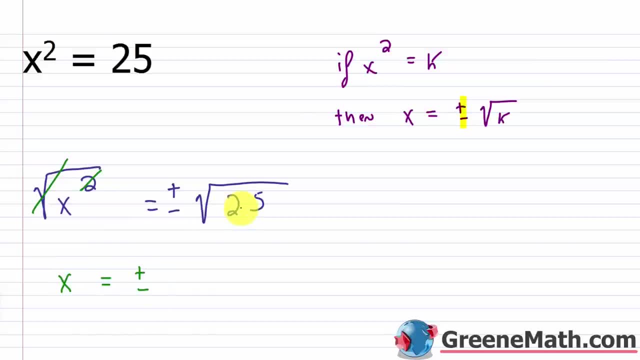 Then it equals plus or minus the square root of 25, we know at this point is 5. 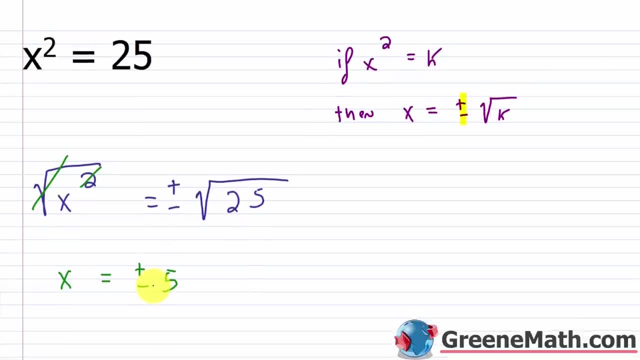 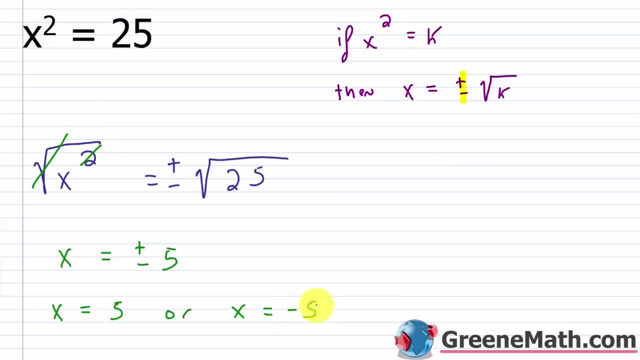 So what this notation is telling me is I have, again, two solutions. x can be equal to 5, or x could be equal to negative 5. And you can easily see if I plugged in a 5 here, 5 squared would be 25. 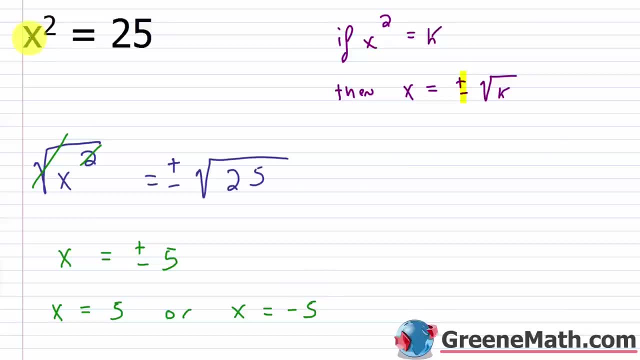 If I plugged in a negative 5, negative 5 inside a parenthesis squared would also be 25. All right, let's take a look at another easy one. 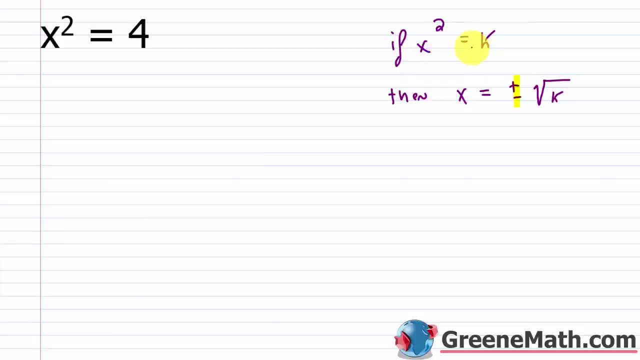 So again, if x squared, equals k and k is positive, then x equals plus or minus the square root of k. 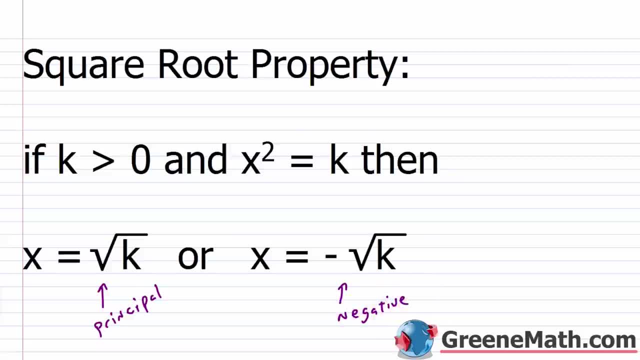 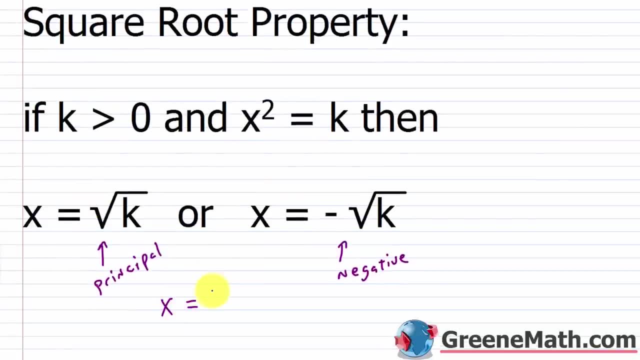 the negative square root of k. And generally what we do to save space is we'll write x is equal to the positive or principal square root of k, and then we put the negative underneath and then we write square root of k. So x equals plus or minus. 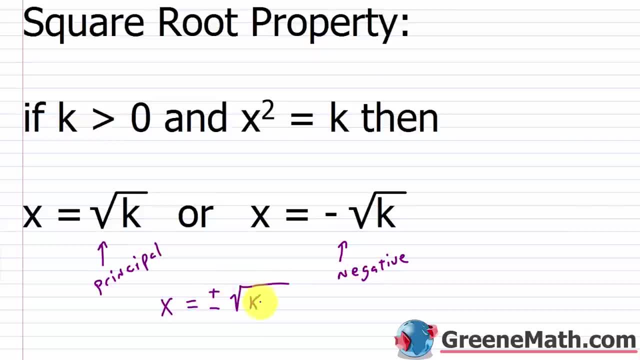 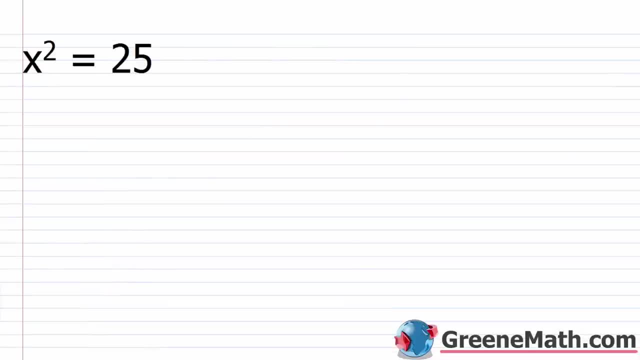 that's how it's read: plus or minus the square root of k. This is just a compact way to write this, Okay, so let's take a look at an easy one. So we have x squared equals 25.. So again, 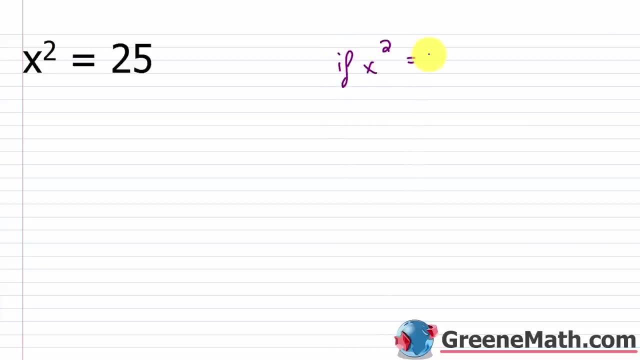 if x squared is equal to k and k is greater than 0, then x is equal to plus or minus the square root of k. So I'm going to do that over here. I'm going to take the square root of each side. 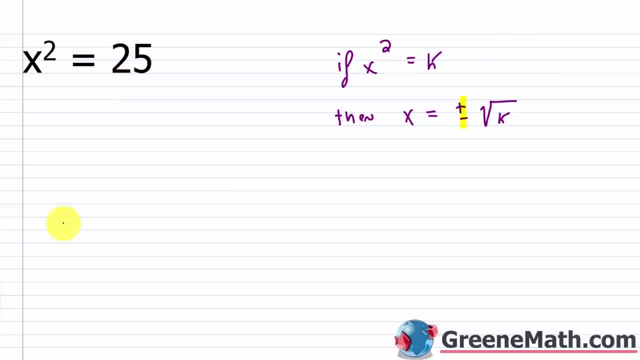 but again I've got to account for the positive and the negative version. So let's write that down here. So we'll have: x squared is equal to 25, and I'm going to take the square root of this side and then over here. 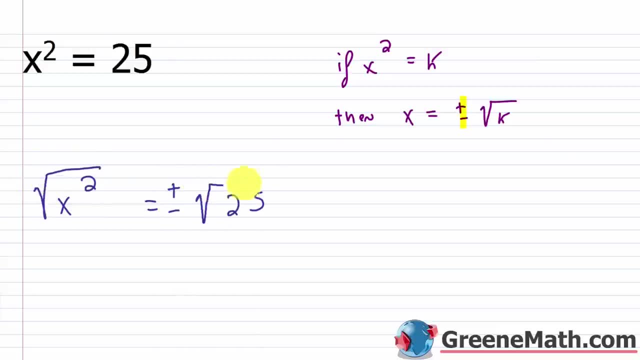 I'm going to put plus or minus the square root of this side. So we know at this point that this cancels with this and we'll have just x. Then it equals plus or minus the square root of 25. we know at this point. 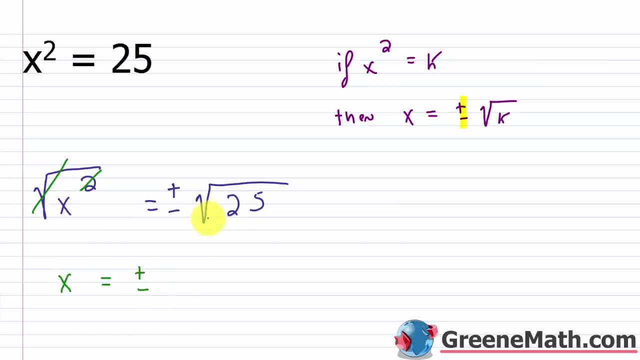 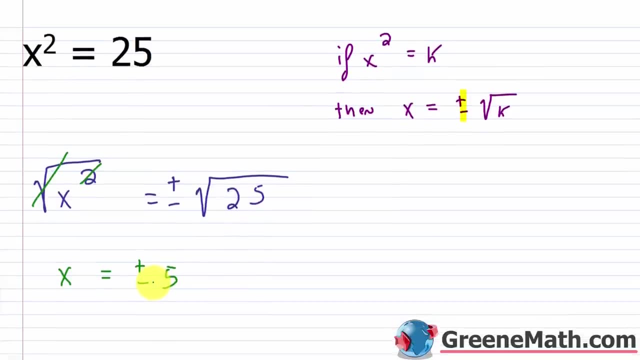 is 5.. So what this notation is telling me is I have again two solutions: x can be equal to 5, or x could be equal to negative 5.. So what this notation is telling me is I have again: 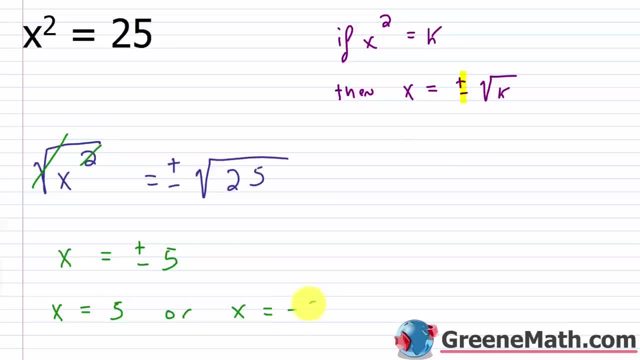 two solutions: x can be equal to 5, or x could be equal to negative 5.. And you can easily see: if I plugged in a 5 here, 5 squared would be 25.. If I plugged in a negative 5,, 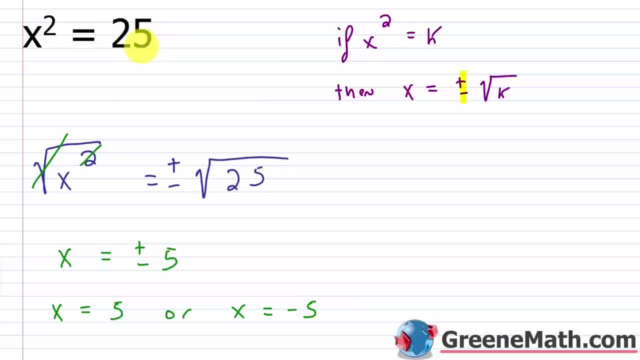 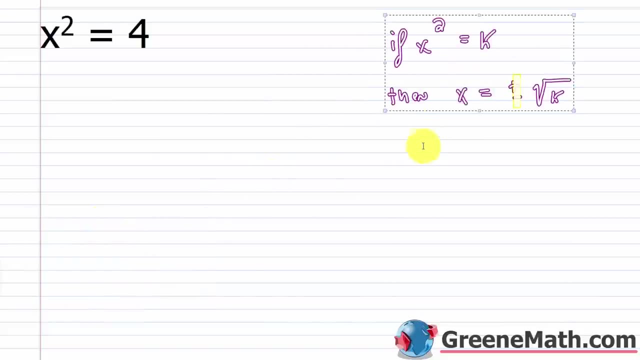 negative 5 inside a parenthesis- squared would also be 25.. All right, let's take a look at another easy one. So again, if x squared equals k and k is positive, then x equals plus or minus the square root of k. 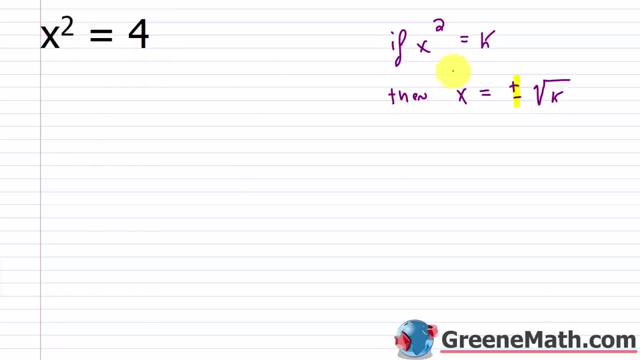 So x squared equals 4.. So we know that we have this same scenario here. So x squared equals 4.. I'm going to take the square root of this side and then over here I'm going to put plus or minus the square root. 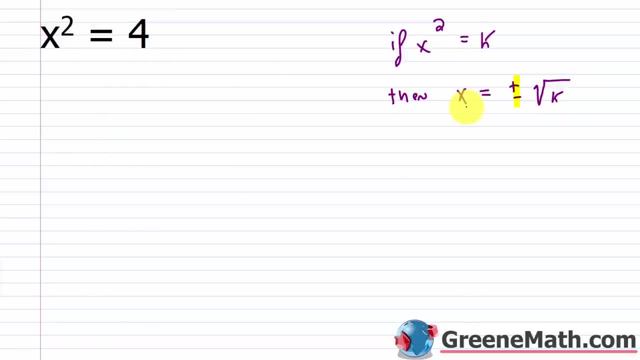 So x squared equals 4. So we have this same scenario here. So x squared equals 4. 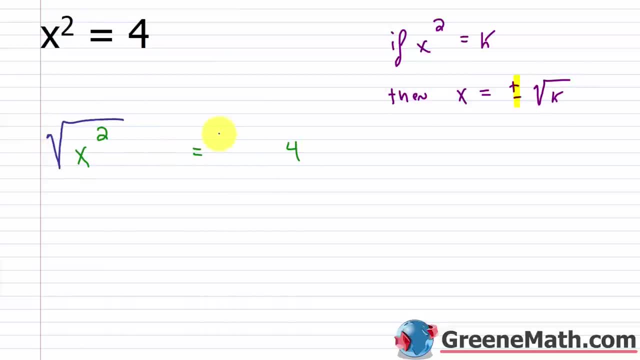 I'm going to take the square root of this side, and then over here I'm going to put plus or minus the square root of this. 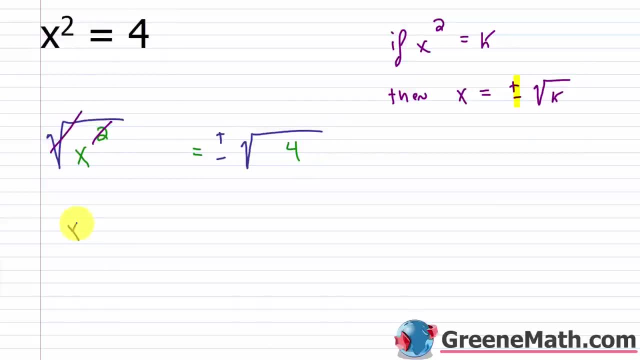 So this cancels with this, and I just have x, 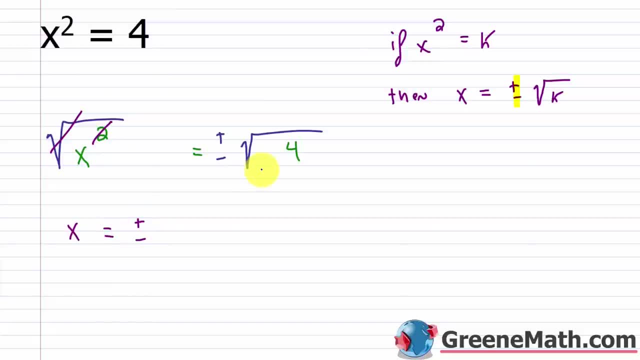 and it's equal to plus or minus, the square root of 4. Square root of 4 is 2. 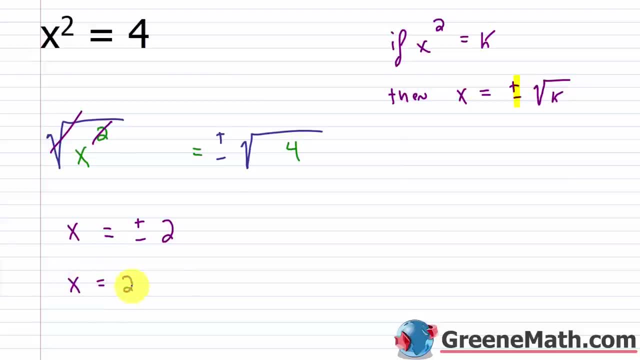 So again, this tells me I have two solutions. x is equal to 2, or x is equal to negative 2. 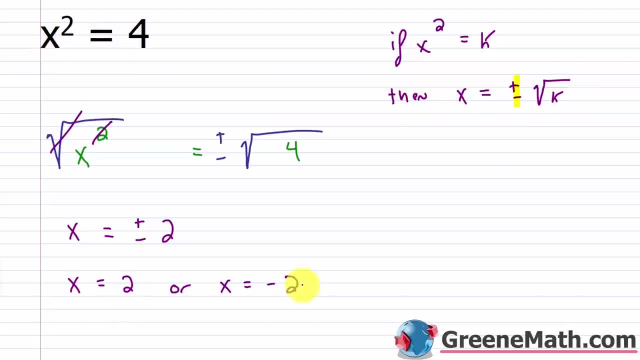 And again, if you plug this in, 2 squared is obviously 4, and then negative 2, negative 2 times negative 2, or negative 2 squared, is also 4. 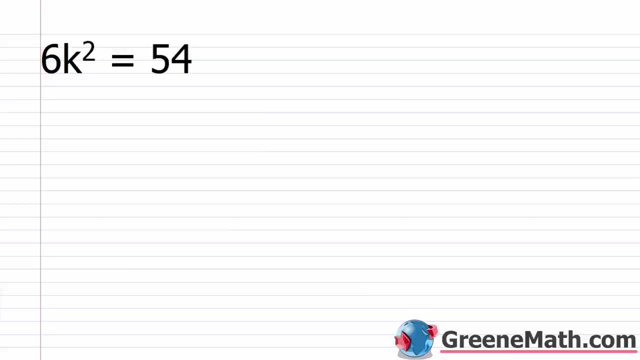 All right, so let's look at one that's a little bit more complex. So let's say you're in this section on the square root property, and you turn to a problem that looks, like this. 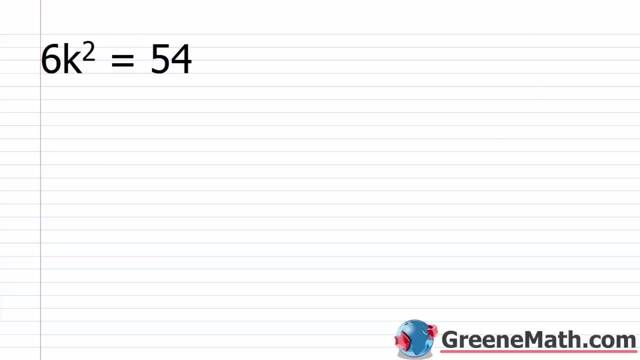 6k squared equals 54. And you're thinking, okay, well, 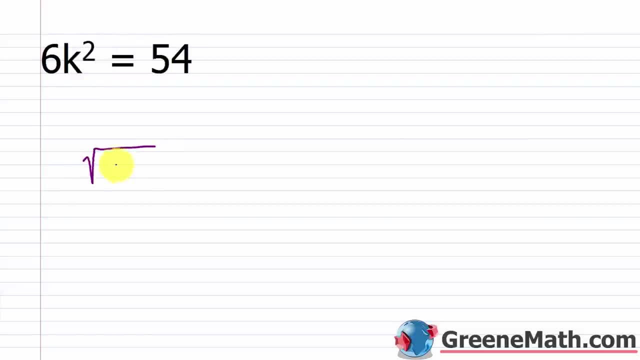 I have a square here. So let me take the square root of 6k squared equals 54 plus or minus the square root of that. 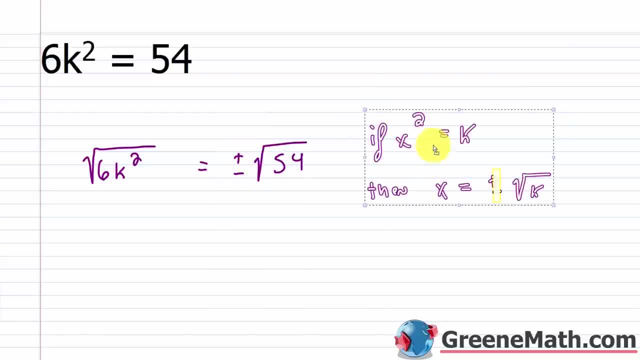 Is that going to get you where you need to go? No, it is not. 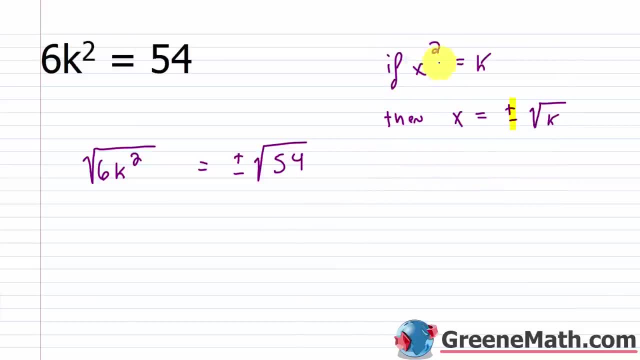 So by the formula, what you want is something squared equals to some number. 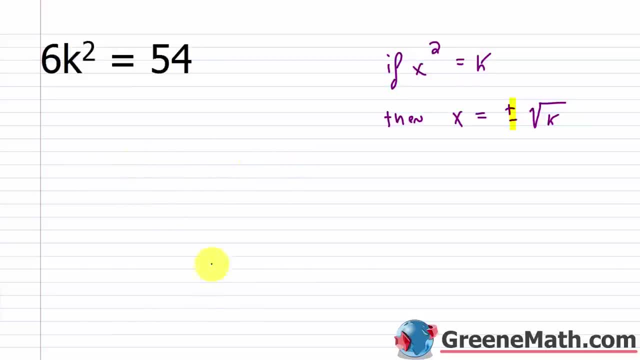 Now, we don't have a perfect square because 6 is not, a perfect square. 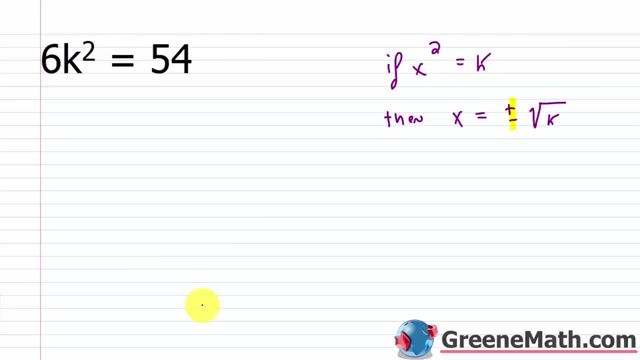 So what you want to do is think about basic things that you could do to get a perfect square over here. 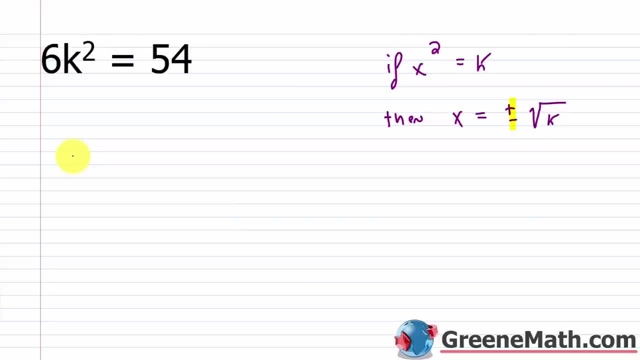 Now, we're going to get into some very complicated examples of this in the next section where we talk about completing the square. 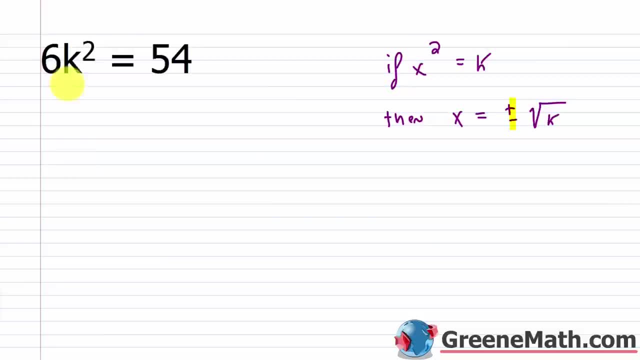 But for right now, I want you just to think about what can I do to get k squared by itself? Well, I can divide both sides of the equation by 6. 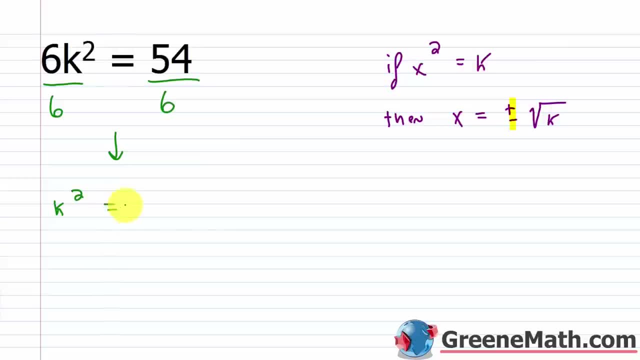 This would yield k squared, plus or minus the square root of 9. 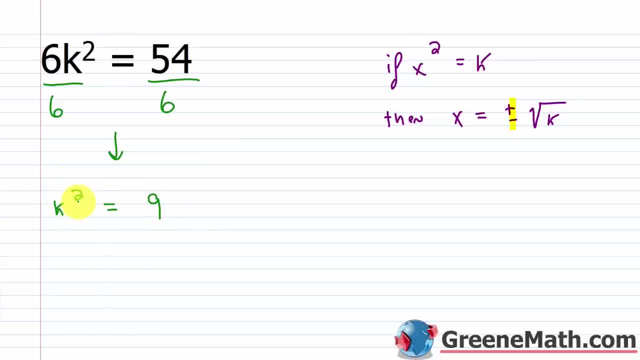 So now I have a perfect square on the left. And what's going to happen is, 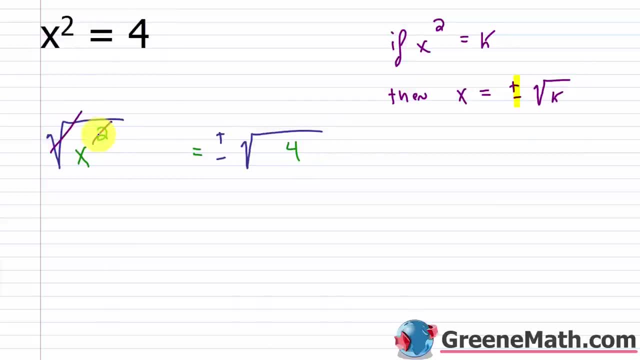 of this. So this cancels with this and I just have x and it's equal to plus or minus the square root of 4.. The square root of 4 is 2.. So again, this tells me I have two solutions. 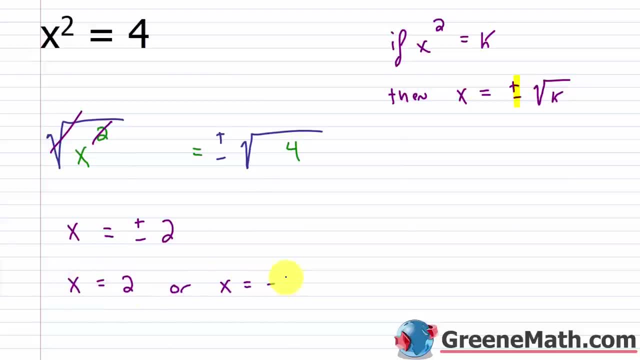 x is equal to 2, or x is equal to negative 2.. And again, if you plug this in, 2 squared is obviously 4, and then negative 2, negative 2 times negative 2, or negative 2 squared. 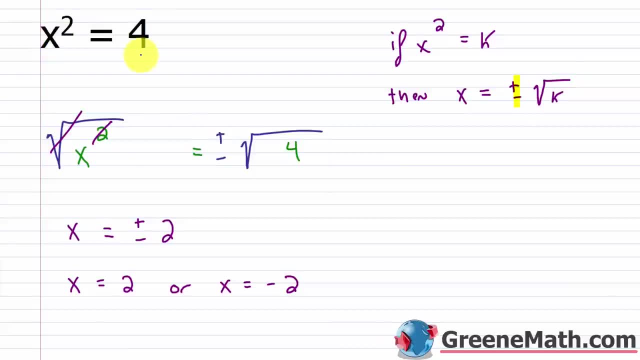 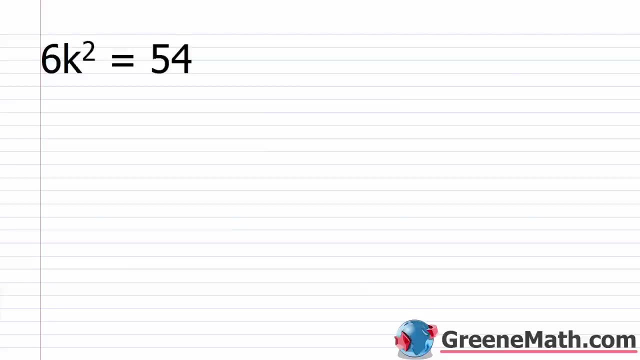 is also 4.. All right, so let's look at one that's a little bit more complex. So let's say you're in this section on the square root property and you turn to a problem that looks like this: 6k squared. 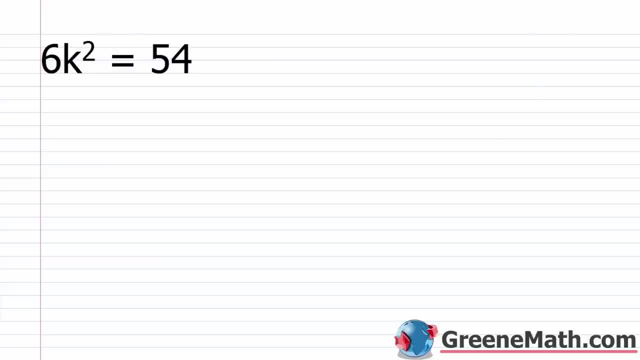 equals 54.. And you're thinking, okay, well, I have a square here, so let me take the square root of 6k. squared equals 54, plus or minus the square root of that. Is that going to get you where you need? 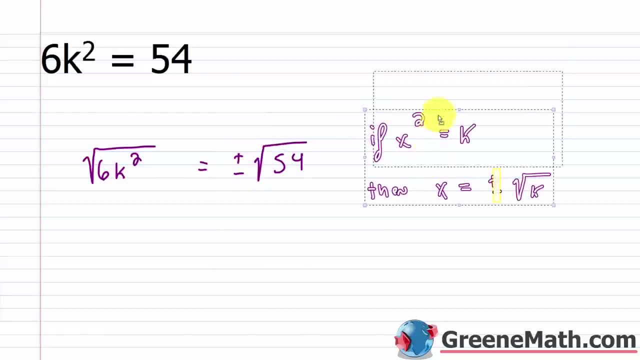 to go. No, it is not. So by the formula. what you want is something squared equals to some number. Now, we don't have a perfect square, because 6 is not a perfect square. So what you want to do is: 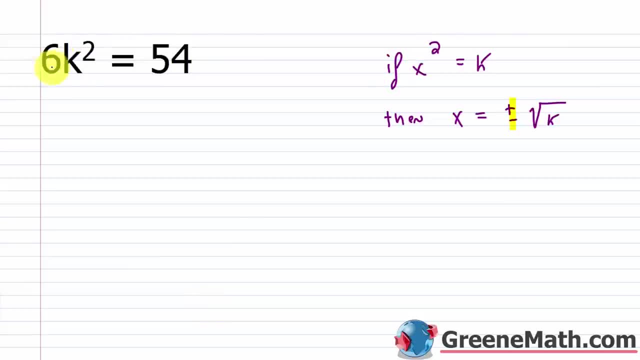 think about basic things to get a perfect square over here. Now. we're going to get into some very complicated examples of this in the next section, where we talk about completing the square, But for right now, I want you just to think about what can. 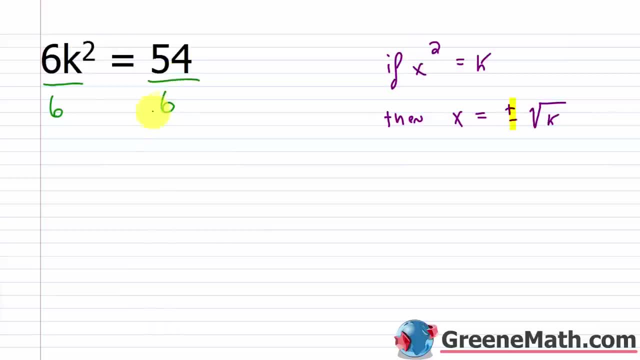 I do to get k squared by itself. Well, I can divide both sides of the equation by 6. This would yield: k squared is equal to 9.. So what's going to happen is if I take the square root of k squared, 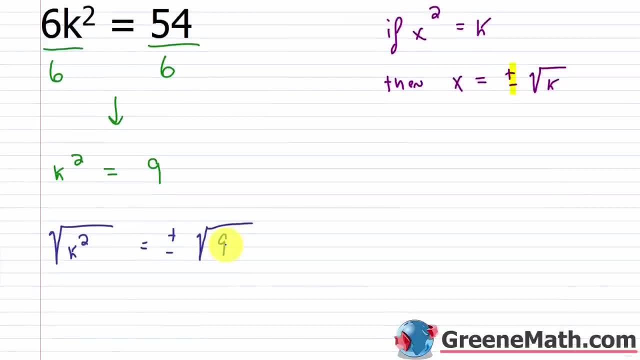 and set this equal to plus or minus the square root of 9, I get my solution. This is going to give me k is equal to plus or minus. square root of 9 is 3.. So this yields k equals 3 and k equals. 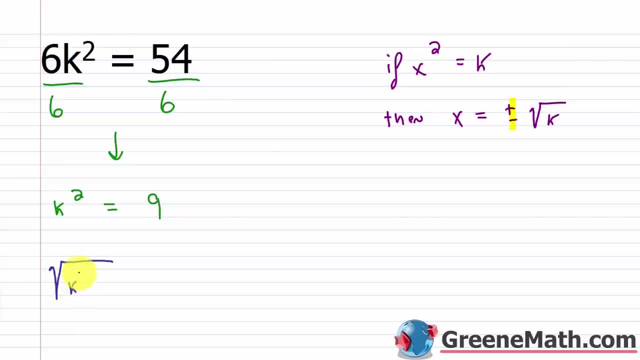 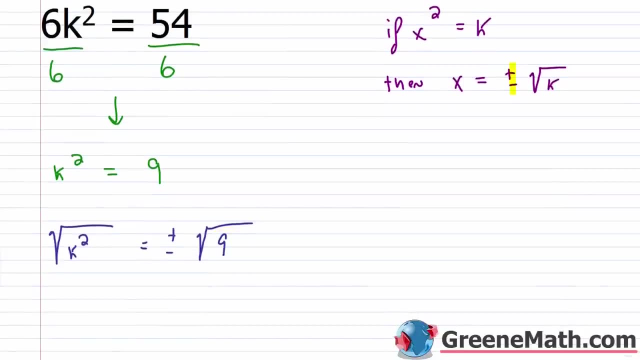 if I take the square root of k squared, and set this equal to plus or minus the square root of 9, I get my solution, right? 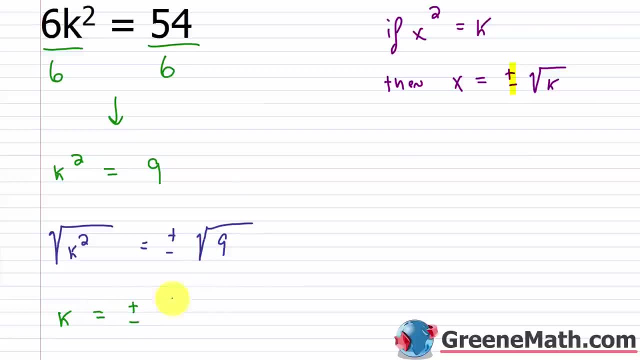 This is going to give me k is equal to plus or minus square root of 9 is 3. So this yields k equals 3 or k equals negative 3. 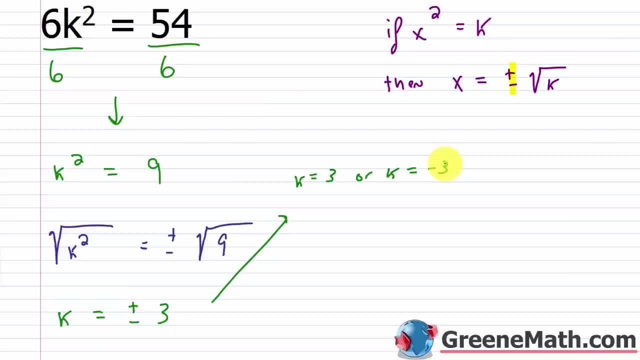 So does this work as a solution? Well, let's erase all of this over here. And let's plug in. 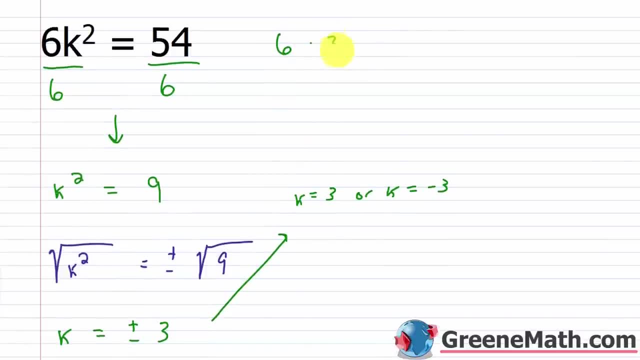 So if I had 6 times 3 squared, would that equal 54? 3 squared is 9. 9 times 6 is 54. So that checks out. 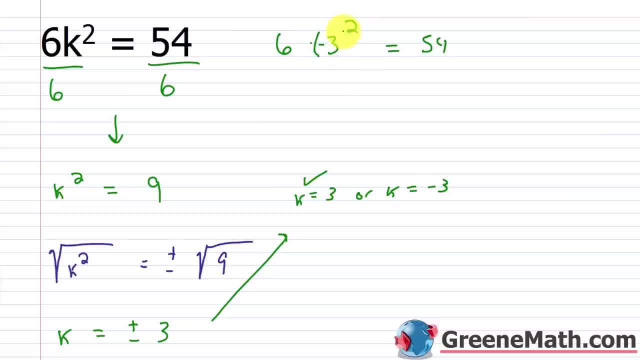 What if I had 6 times negative 3 inside a parentheses squared? Well, it's the same thing. 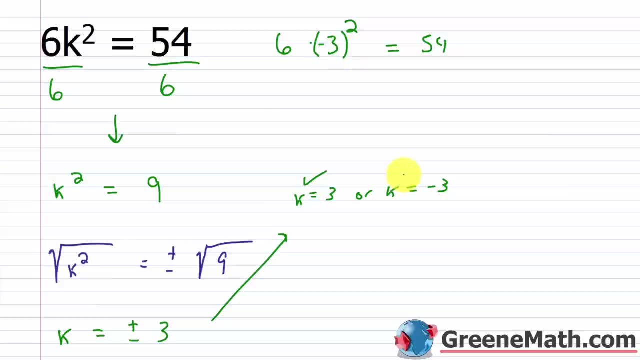 I'd end up with 6 times 9. 6 times 9 is again 54. So this checks out. 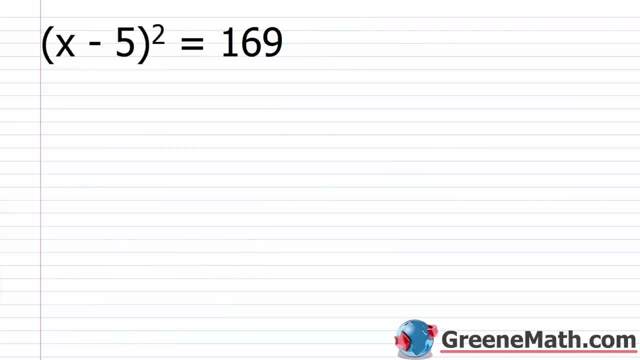 Now, additionally, we can use this rule when we have a squared binomial. 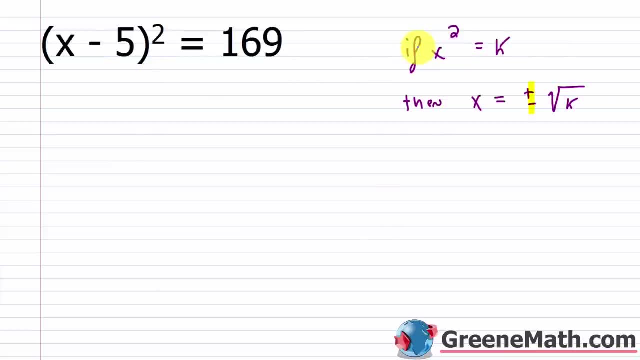 So I just want you to pretend that you're substituting in for that x. You're substituting this whole thing. So if x minus 5, 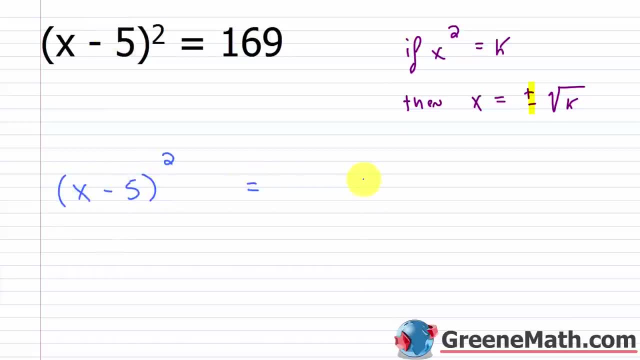 that quantity squared is equal to 169. 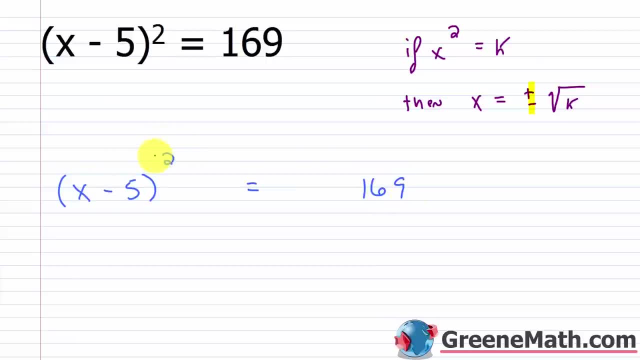 Again, to get x by itself, I've got to first get rid of this squared here. So let me take the square root of this side and then plus or minus. The square root of this side. Now, it's going to be a little bit more work in terms of simplification because now this will cancel with only this. And I'm left with this x minus 5 here. 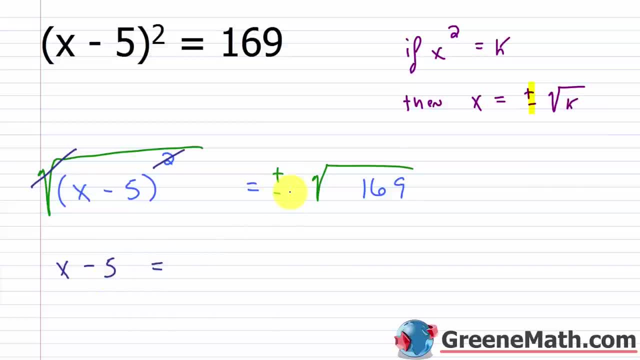 And this equals plus or minus the squared of 169, which is plus or minus 13. 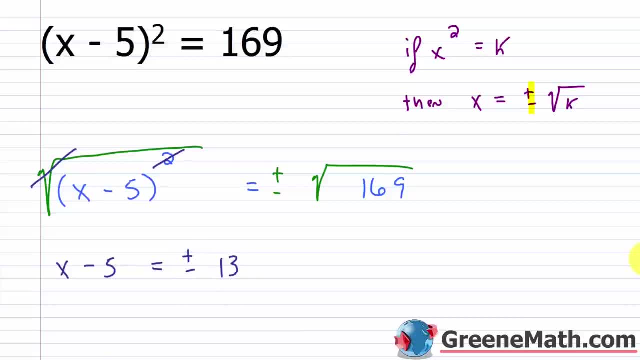 Now, I have two possible scenarios here. So that's where it becomes more work. 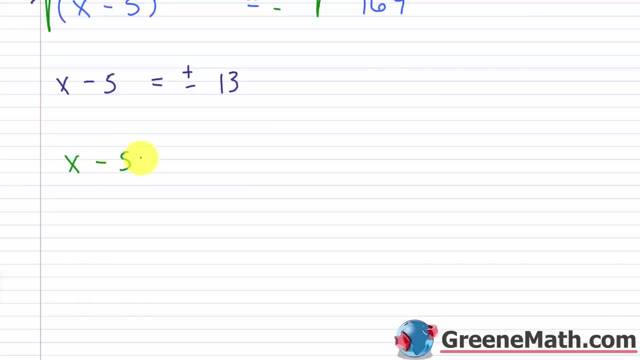 I have to separate this now into x minus 5 is equal to positive 13. Or x minus 5 is equal to negative 13. 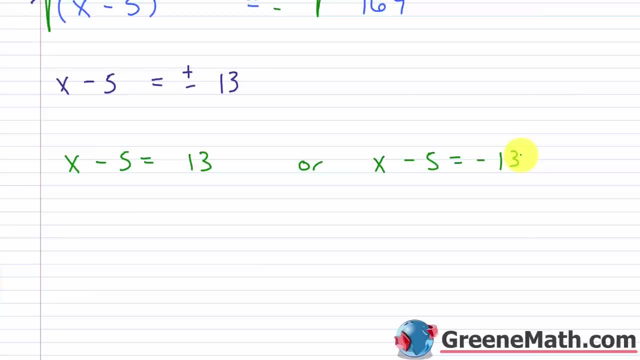 So on these more complex examples, you're going to have more things that you have to do. So let me add 5 to both sides of the equation here. 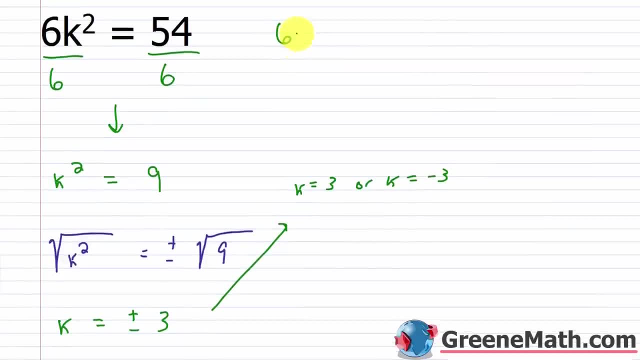 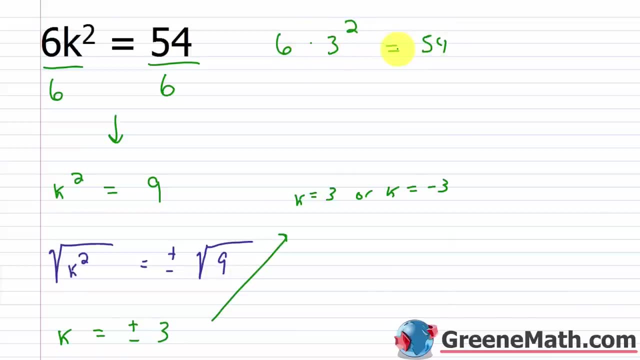 4.. So I can do this over here and let's plug in. So if I had 6 times 3 squared, would that equal 54?? 3 squared is 9.. 9 times 6 is 54.. 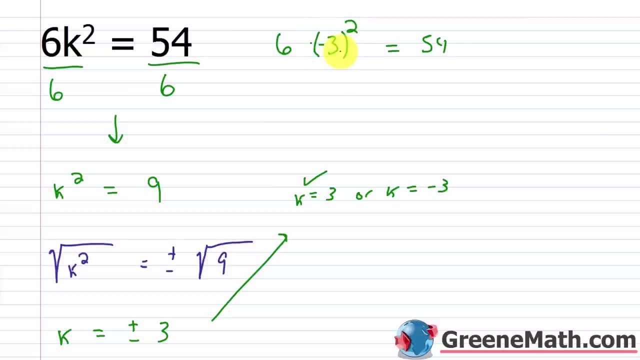 So that checks out. What if I had 6 times negative, 3 inside of parentheses squared? Well, we have a squared binomial. So I just want you to pretend that you're substituting in for that x. You're substituting. 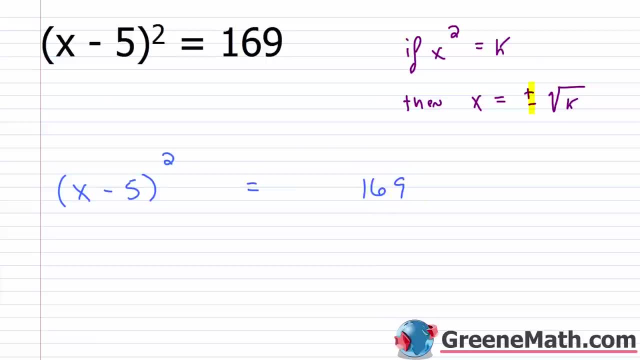 this whole thing. So if x minus 5, that quantity squared is equal to 169.. Again, to get x by itself I've got to use multiplication, because now this will cancel with only this and I'm left with this x minus. 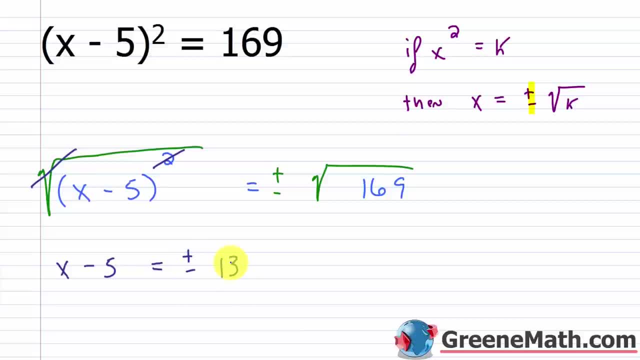 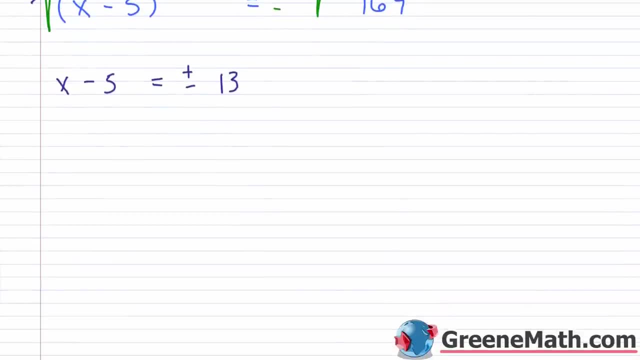 5 here, and this equals plus or minus the squared of 169, which is plus or minus 13.. Now I have two possible scenarios here, So let's go back to the top and we're going to check our solutions. So. 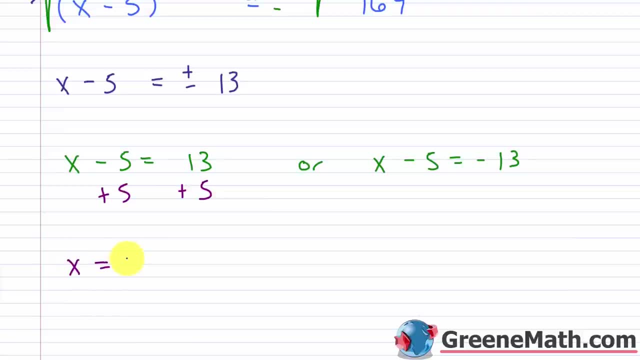 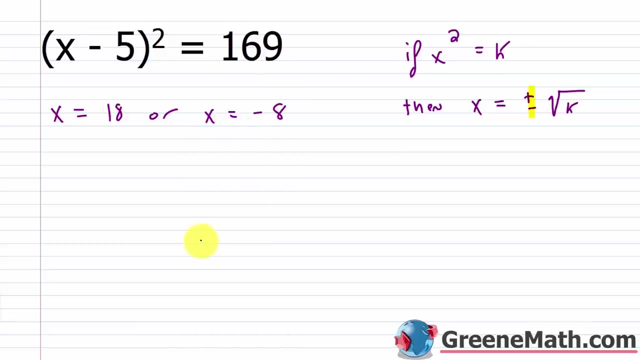 again, we found that x was equal to negative 8.. So let's copy this and we'll go back up to the top and we're going to check our solutions. So let's go back to the top and we're going to. 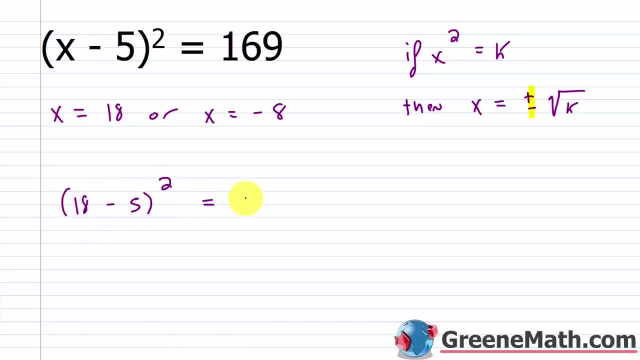 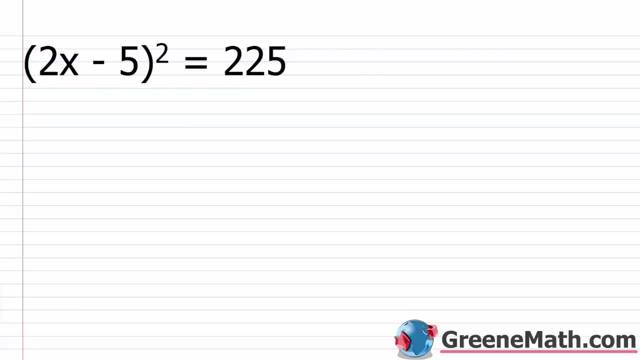 plug in our solutions. So let's plug in our solutions. So let's plug in our solutions. So let's plug in the solutions. So here we posted the solution so that we can model it in a good way. So 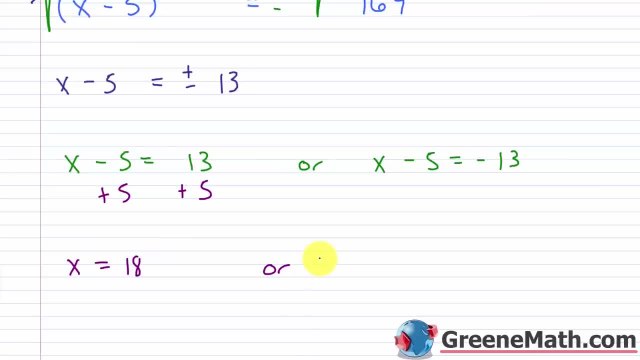 I'm going to get x is equal to 18. Then or let me add 5 to both sides of the equation here. And I'm going to get x is equal to negative 8. 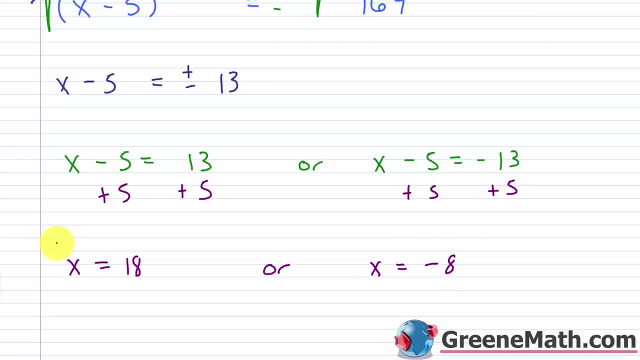 All right, so let's copy this. And we'll go back up to the top. And we're going to get x is equal to negative 8. And we're going to check our solutions. So again, we found that x was equal to 18, or x was equal to negative 8. 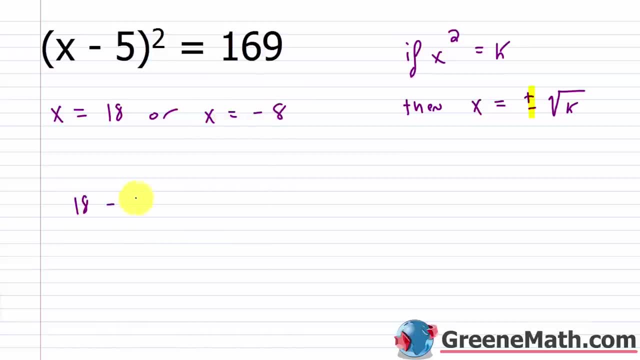 So let's start by plugging in an 18. So if I had 18 minus 5, and that amount was squared, would this equal 169? 18 minus 5 is 13. So we'd have 13 squared equals 169. So that checks out. 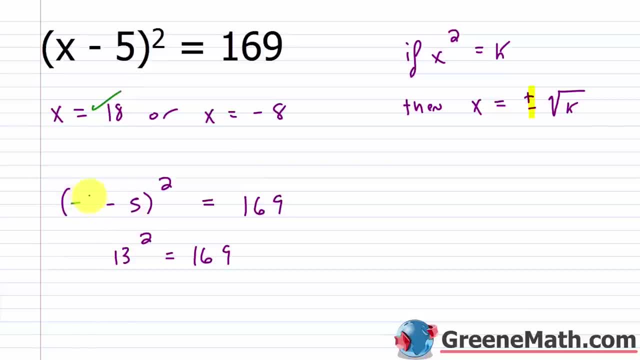 For the next one, we have negative 8. So if I plugged in a negative 8 there, so we have negative 8 minus 5, that's negative 13. 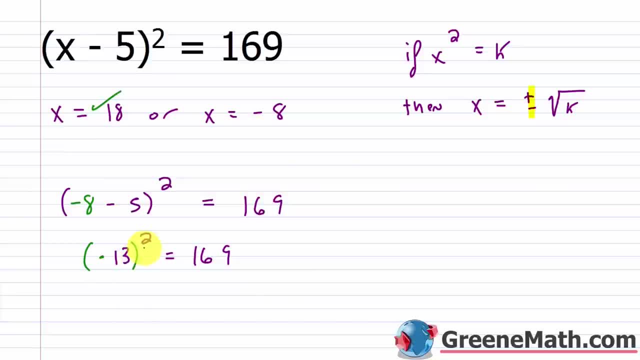 So if I had negative 13 inside of parentheses and it was squared, that would also give me positive 169. 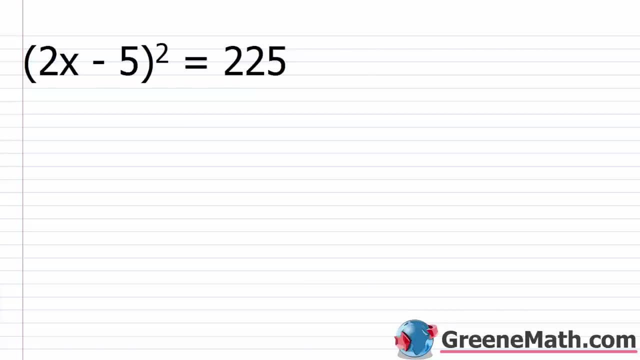 All right, let's try another one like that. So let's suppose we had the quantity 2x minus 5, and that's squared. 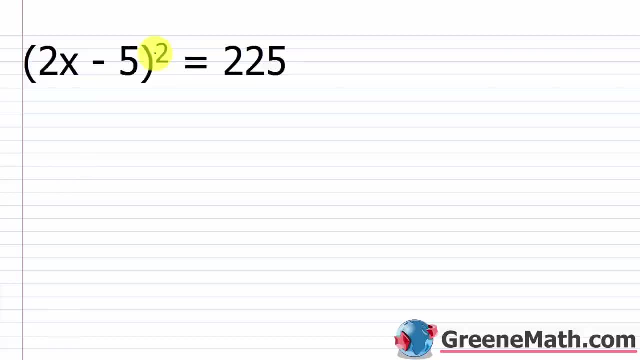 This equals 225. So again, simple setup. I'm just trying to get rid of the squared right there. 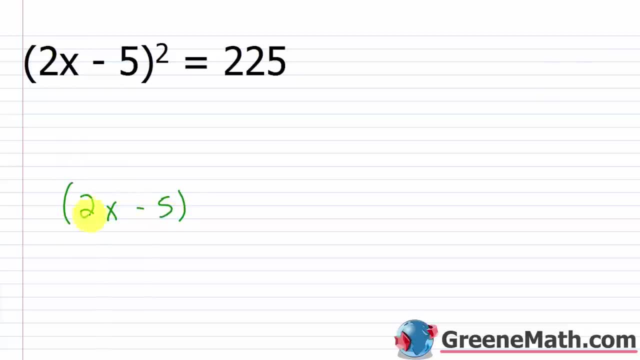 So I can get x by itself in the end. So let's rewrite this. 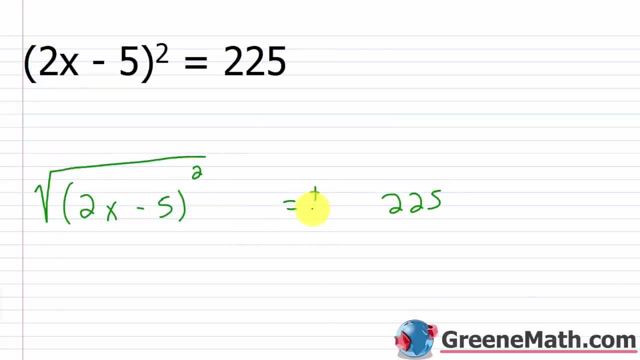 I'm going to take the square root of this side, and I'm going to put plus or minus the square root of this side. 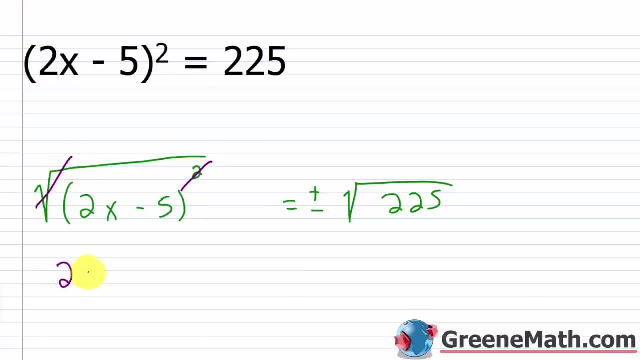 So then this will cancel with this, and I'm left with 2x minus 5 is equal to plus or minus the square root of 225. 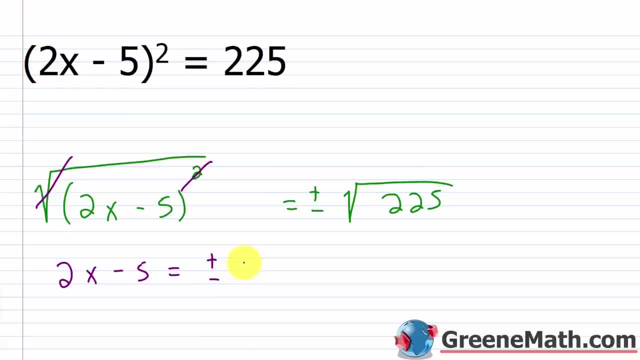 The square root of 225, in case you don't know this, is 15. 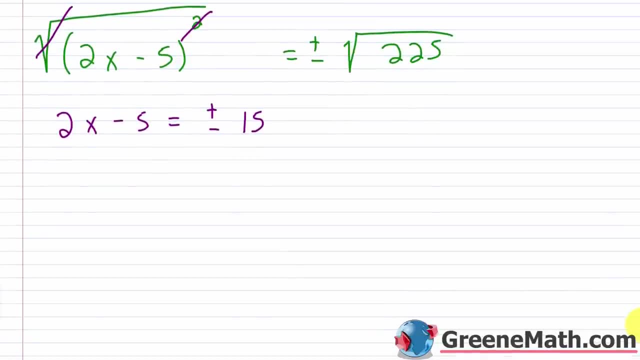 So this sets up two different equations to solve. You're going to have 2x minus 5 is equal to positive 15. 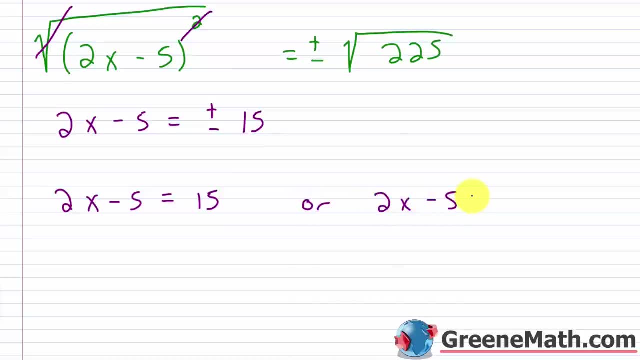 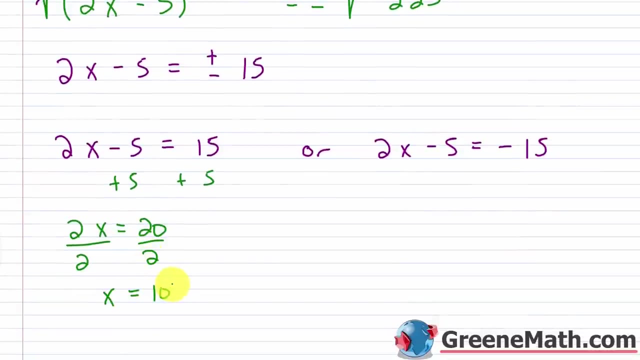 Then or, you're going to have 2x minus 5 is equal to negative 15. So let's go ahead and add 5 to both sides of the equation here. You'll have 2x is equal to 20. Divide both sides of the equation by 2. You're going to get x is equal to 10, okay? 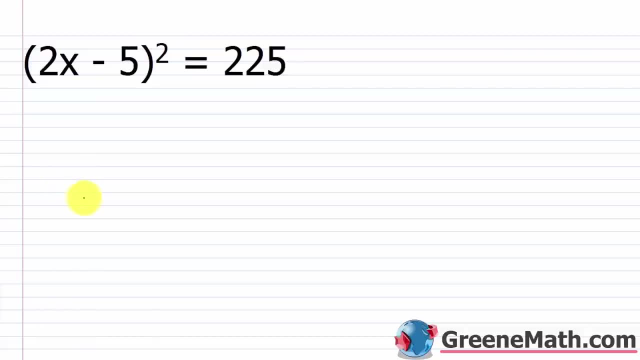 when you try to take all the solutions out on the machine, take the square root of this side and I'm going to put plus or minus the square root of this side, so then this will cancel with this and I'm left with 2x minus 5 is equal to plus or minus the. 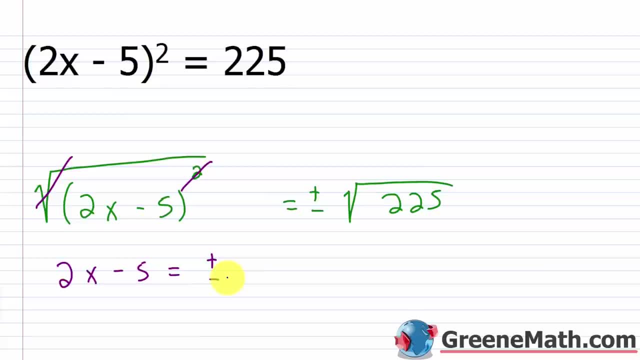 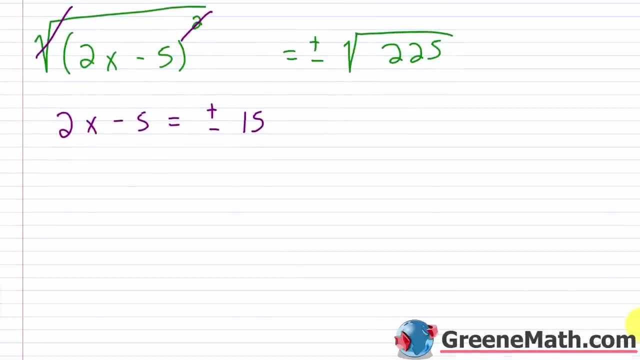 square root of 225. the square root of 225, in case you don't know, this is 15. so this sets up two different equations to solve. you're going to have 2x minus 5 is equal to positive 15, then, or you're going to have 2x minus 5 is equal to negative 15, so let's go ahead and add 5 to both. 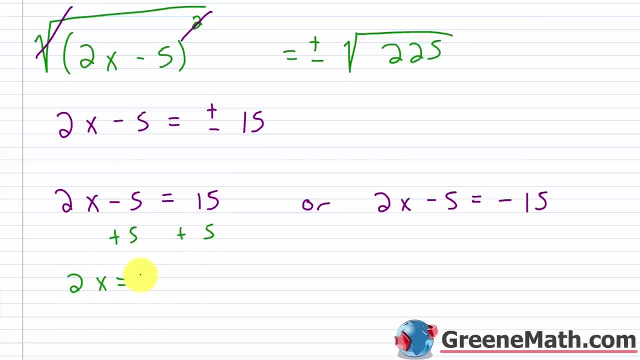 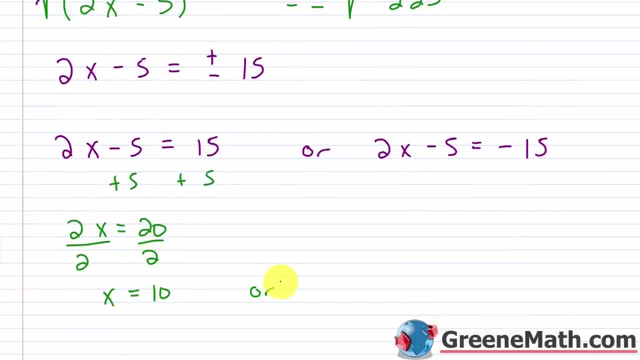 sides of the equation. here you'll have: 2x is equal to 20. divide both sides of the equation by 2, you're going to get x is equal to 10. okay then. or we have plus 5 on both sides. here we'll have: 2x is equal to negative 10. let me scroll down a little bit. we divide both sides by 2. 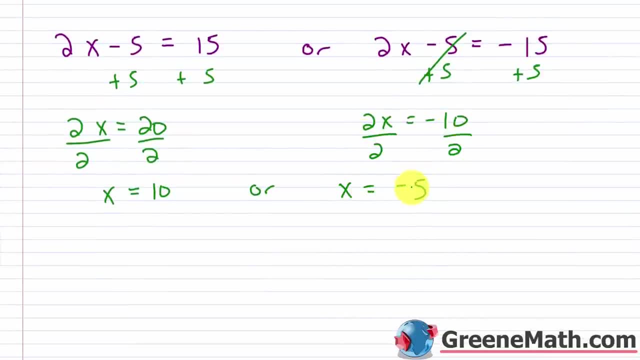 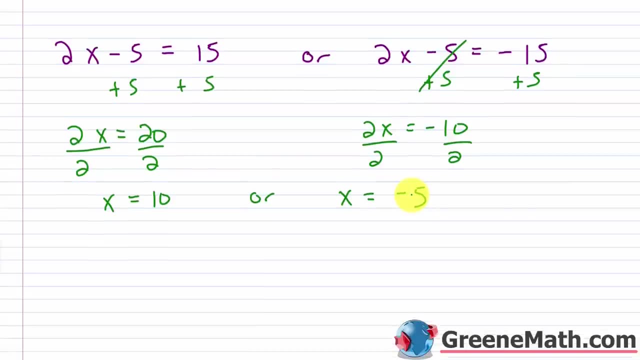 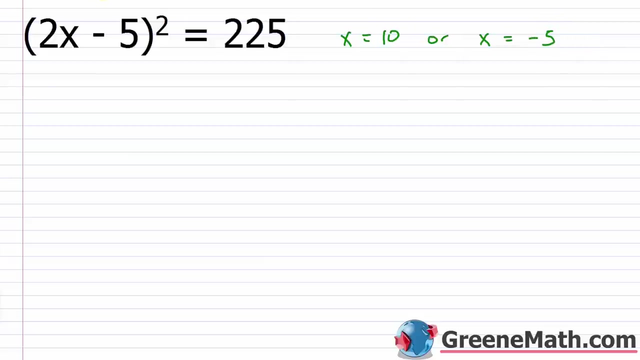 we're going to get x is equal to negative 5. so here's my two solutions: x equals 10 or x equals negative 5. so let's erase everything and check so again: x equals 10 or x equals negative 5. okay, so we'll have inside of parentheses, 2 times 10 minus 5 and this is squared. this equals 225. 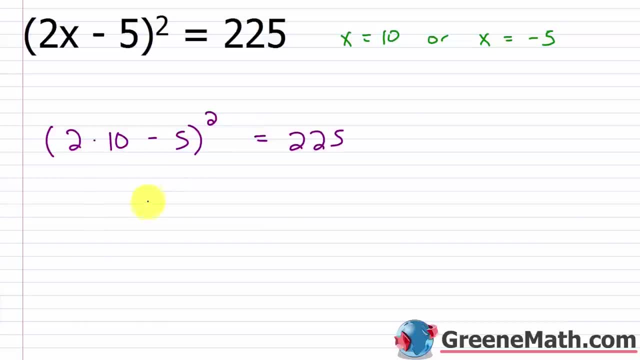 is 20. 20 minus 5 is 15. 15 squared is 225. so this checks out. what about? x equals negative 5. so if we multiply there 2 times, negative 5 is negative 10. negative 10 minus 5 is negative 15. 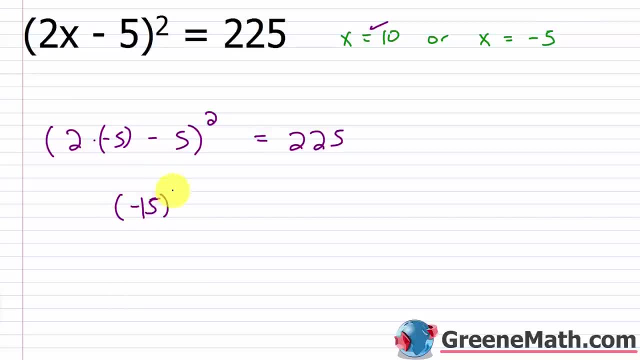 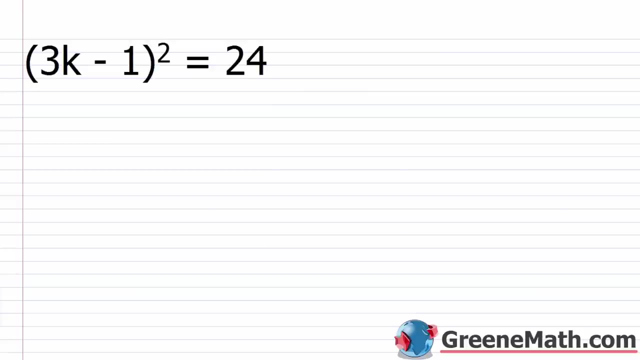 so you'd end up with negative 15 squared is equal to 225, and that also gives me a true statement. you'll get 225 equals 225, and so this checks out as well. all right, for the next one, we have 3k minus 1. that quantity squared is equal to 24, so again, 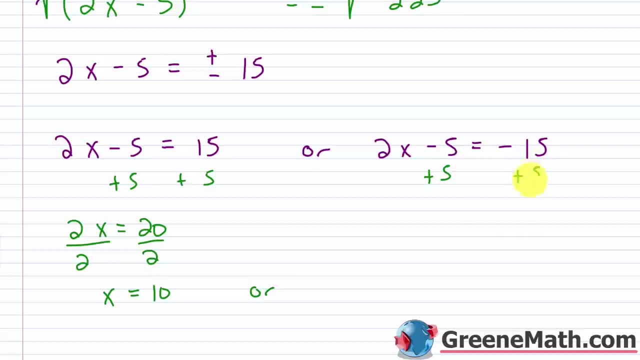 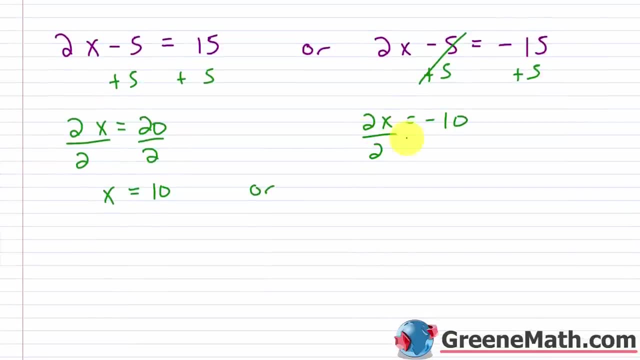 Then or, we have plus 5 on both sides here. We'll have 2x is equal to negative 10. Let me scroll down a little bit. We divide both sides by 2. We're going to get x is equal to negative 5. 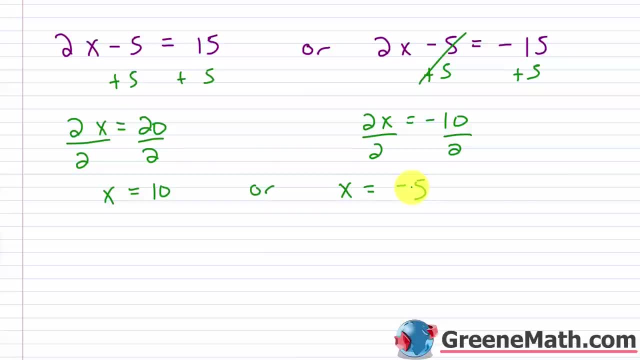 So here's my two solutions, x equals 10 or x equals negative 5. So let's erase everything and check. 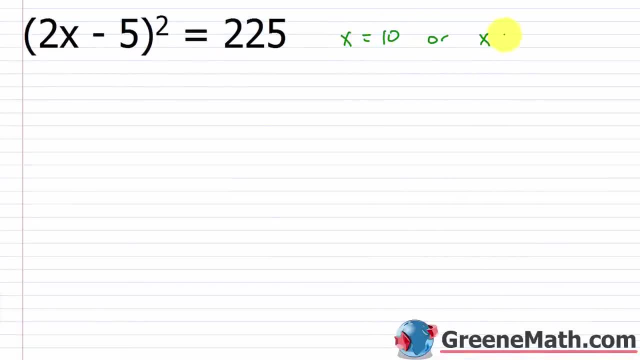 So again, x equals 10 or x equals negative 5. 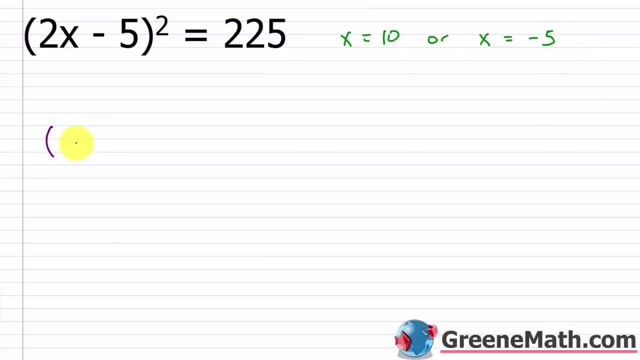 Okay, so we'll have inside of parentheses, 2 times 10 minus 5, and this is squared, this equals 225. 2 times 10 is 20, 20 minus 5 is 15, 15 squared is 225. So this checks out. What about x equals negative 5? 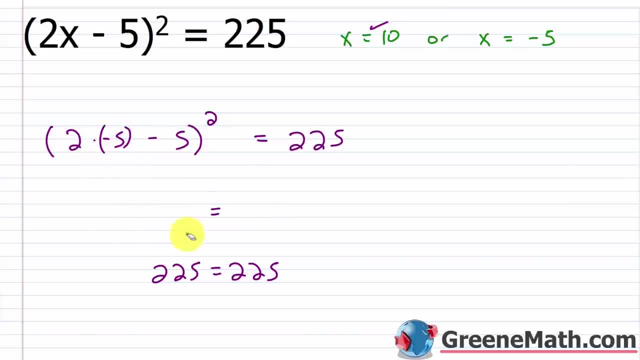 So if we multiply there, 2 times negative 5 is negative 10, negative 10 minus 5 is negative 15, so you'd end up with negative 15 squared is equal to 225, and that also gives me a true statement. 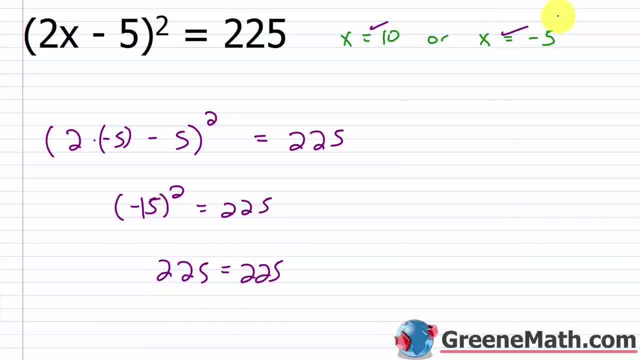 You'll get 225 equals 225, and so this checks out as well. 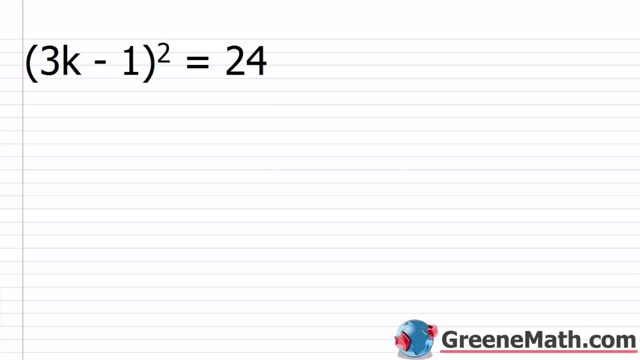 All right, for the next one, we have 3k minus 1, that quantity squared is equal to 24. So again, I'm going to take 3k minus 1, this is squared, equals 24. I'm going to take the square root of this side so that this will cancel with this, and I'm left with this. So I've got 3k minus 1 over here, and then over here, I've got my plus or minus the square root of 24. So equals plus or minus the square root of 24. 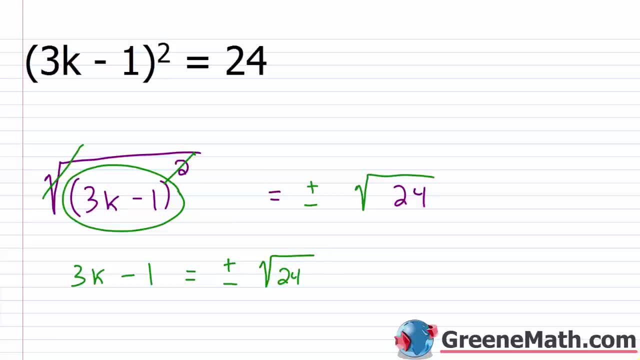 Now, here we're going to have one that's a little bit more tedious, and the reason is that 24 is not a perfect square. 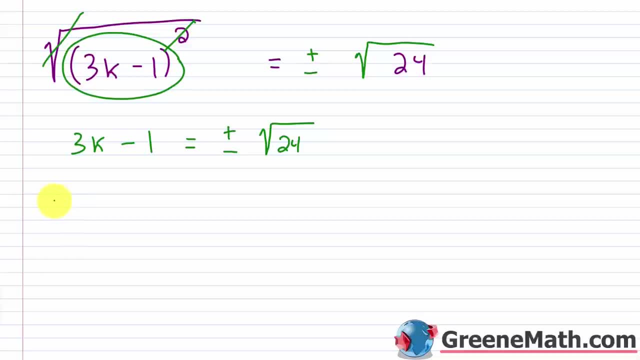 So we have to do some simplification here. So let's write 3k minus 1 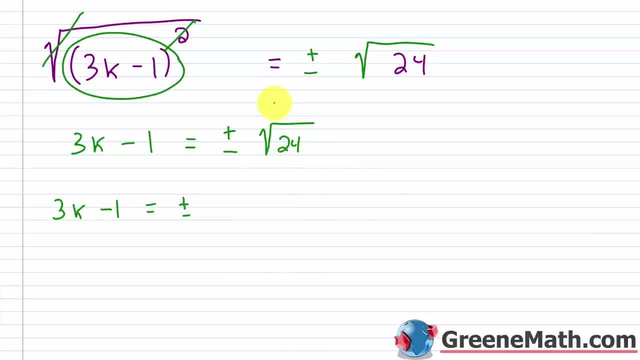 is equal to plus or minus. If I think about the square root of 24, 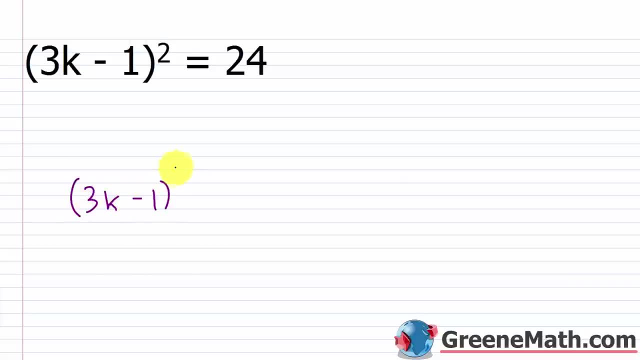 i'm going to take 3k minus 1. this is, squared, equals 24. i'm going to take the square root of this side so that this will cancel with this and i'm left with this. so i've got 3k minus 1 over here, and then over here i've got my plus or minus the square root. 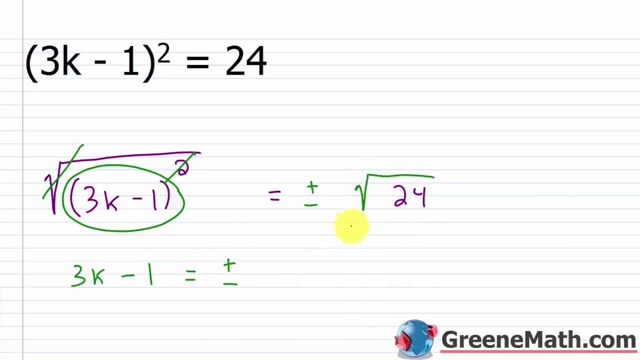 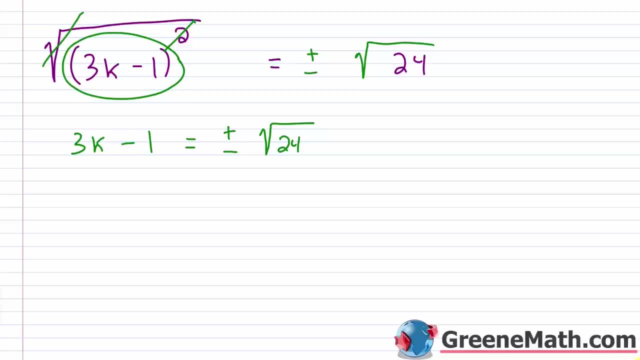 of 24, so equals plus or minus the square root of 24. now here we're going to have one that's a little bit more tedious, and the reason is that 24 is not a perfect square, so we have to do some simplification here. so let's write: 3k minus 1 is equal to. 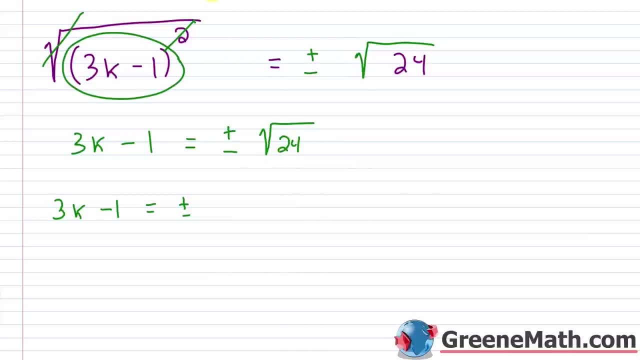 plus or minus. if I think about the square root of 24- I'm just kind of do this off on the side- this is equal to the square root of 4 times the square root of 6, and the square root of 4 is 2. 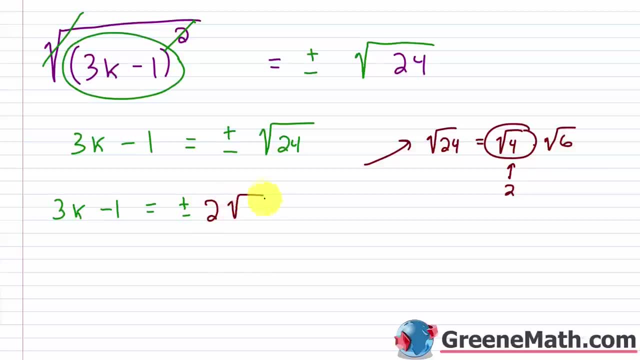 so really this is plus or minus 2 times the square root of 6. now again I've got to set up two different equations. so I would have: 3k minus 1 is equal to 2 times the square root of 6. then, or I'll have: 3k minus 1 is equal to the negative of this, so negative 2 times the square. 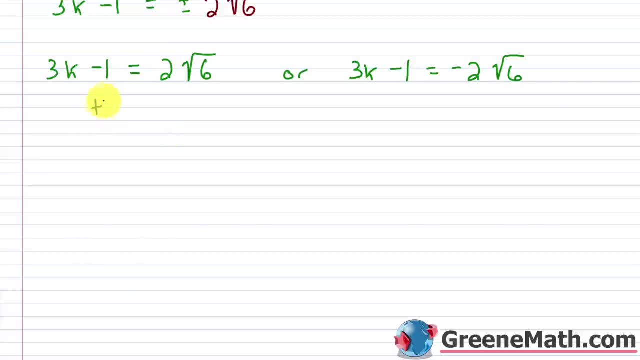 root of 6. all right, so to solve this equation, I would add 1 to each side, so I'll have: 3k is equal to 2 times the square root of 6 plus 1, and then I would divide each side by 3, so I. 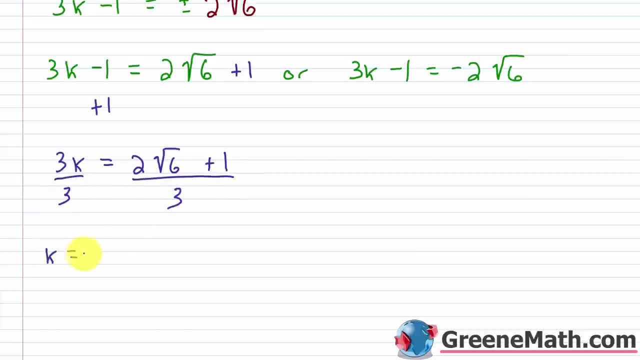 can isolate k and I'm going to have. k is equal to 2 times the square root of 6 plus 1, and then 2 times the square root of 6 plus 1 over 3, and then over here I would add 1 to each side of the. 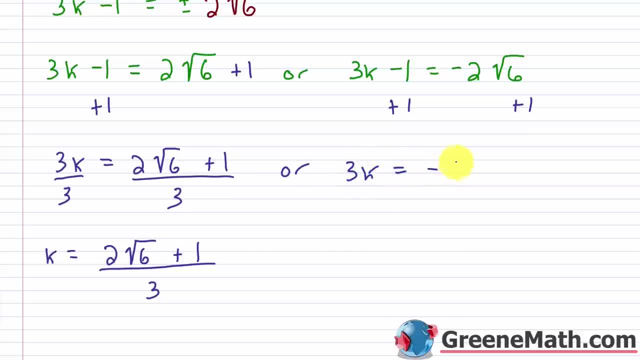 equation. so I'd have: 3k is equal to negative 2 times the square root of 6 plus 1, and then divide again both sides of the equation by 3, so I'll put: or k is equal to negative 2 times the square root. 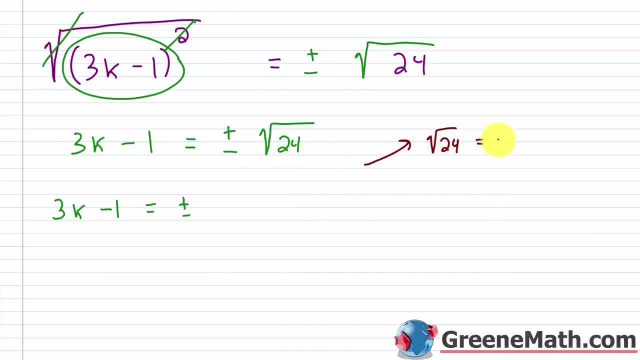 just kind of do this off on the side, this is equal to the square root of 4 times the square root of 6, and the square root of 4 is 2. So really, this is plus or minus 2 times the square root of 6. 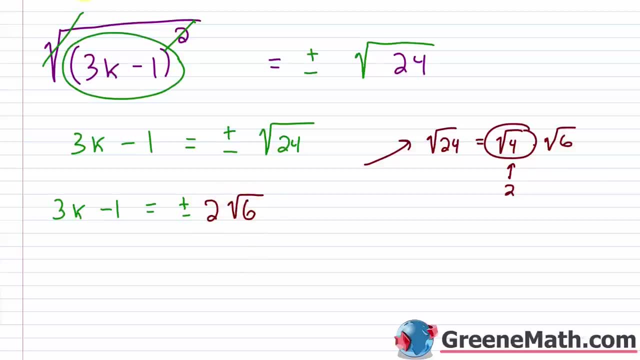 Now, again, I've got to set up two different equations. 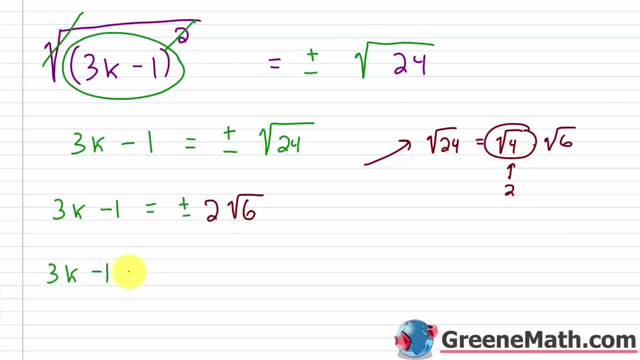 So I would have 3k minus 1 is equal to 2 times the square root of 6, then or I'll have 3k minus 1 is equal to the negative of this, 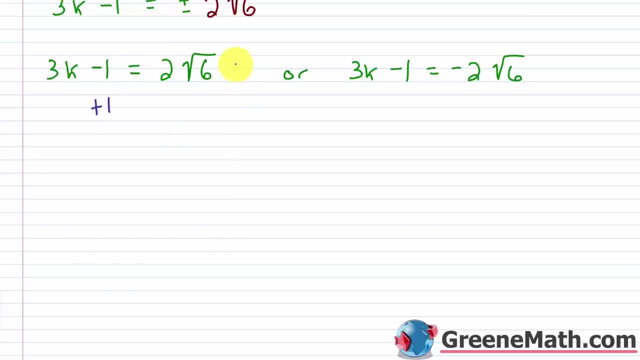 All right, so to solve this equation, I would add 1 to each side. So I'll have 3k is equal to 2 times the square root of 6 plus 1, and then I would divide each side by 3 so I can isolate k, and I'm going to have k is equal to 2 times the square root of 6 plus 1 over 3. And then over here, I would add 1 to each side of the equation. 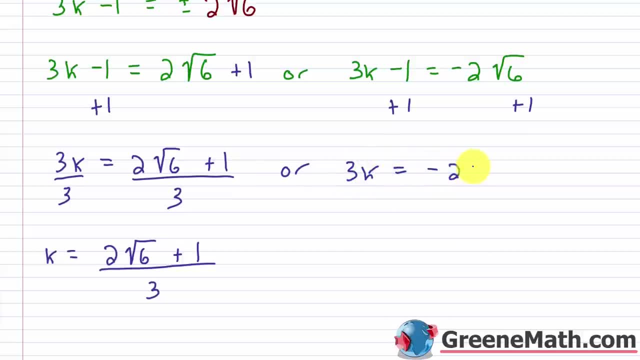 So I'd have 3k is equal to negative 2 times the square root of 6 plus 1, and then divide, again, both sides of the equation by 3. 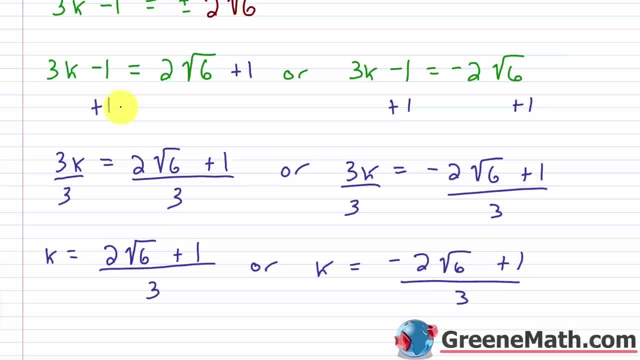 So this is an example of some sloppy solutions that you're going to get. Kind of moving forward. 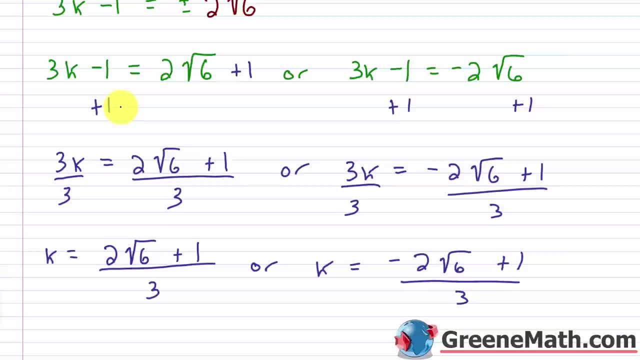 Unfortunately, as you get into higher math, a lot of solutions are much worse than this. And when you go back to try to check things in your original equation, it becomes really, really tedious. 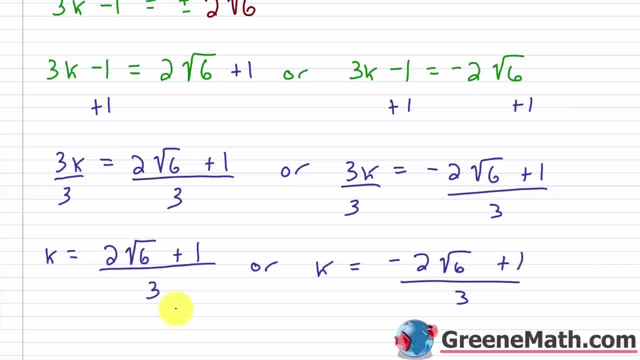 So because this is the last problem, we have some time, we're going to go back and check these two solutions. 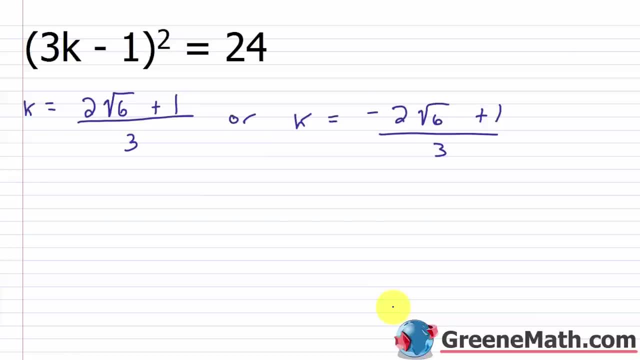 Okay, so plugging this in will be kind of tedious. We're going to have an open parentheses here. We have 3, and then times k. So this is our value for k. So our value for k is 2 times the square root of 6 plus 1 over 3. And then we have minus 1. So then minus 1. 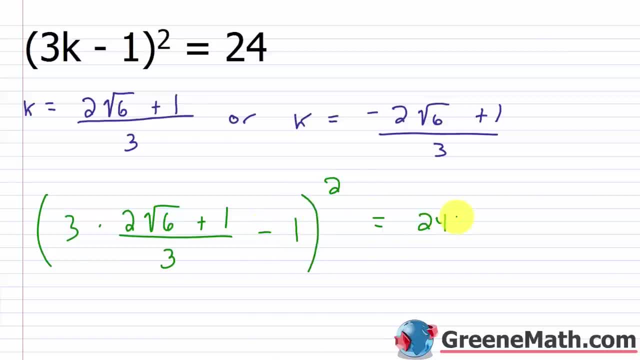 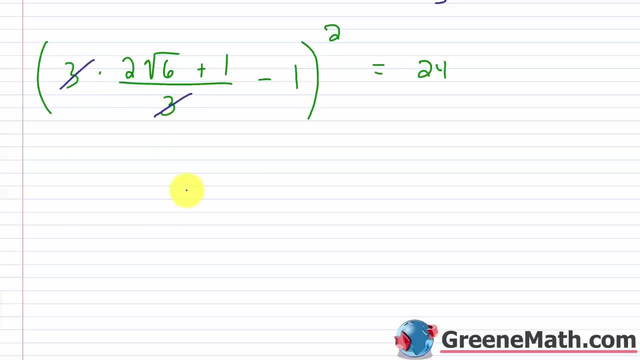 This whole thing is squared, and then it equals 24. So before I square anything, I want you to realize that you can cancel this 3 with this 3. 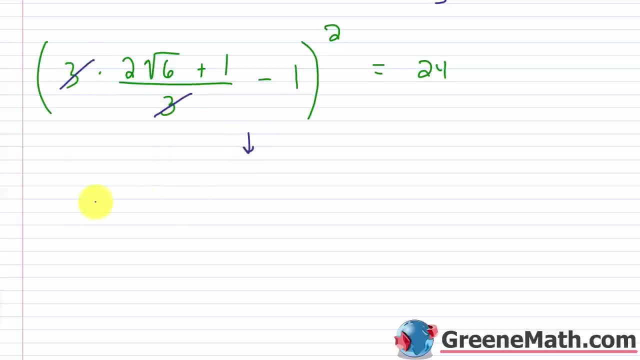 So what would I have then inside? Well, inside the parentheses now, I have 2 times the square root of 6 plus 1 minus 1. 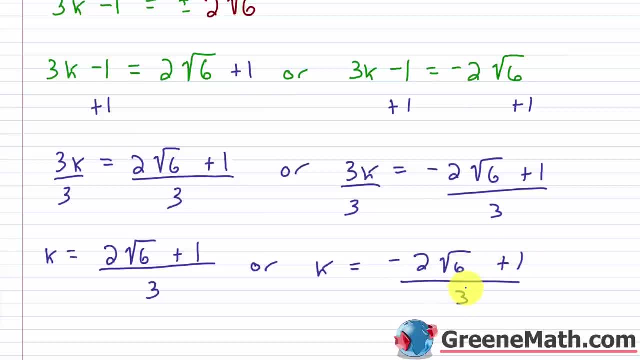 of 6 plus 1 over 3. so this is an example of some sloppy solutions that you're going to get kind of moving forward. unfortunately, as you get into higher math, a lot of solutions are much worse than this and when you go back to try to check things in your original equation, it becomes: 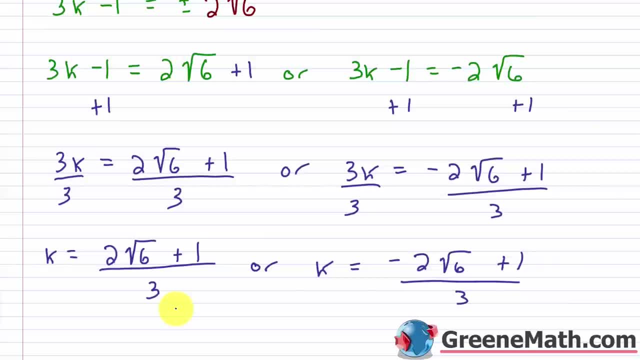 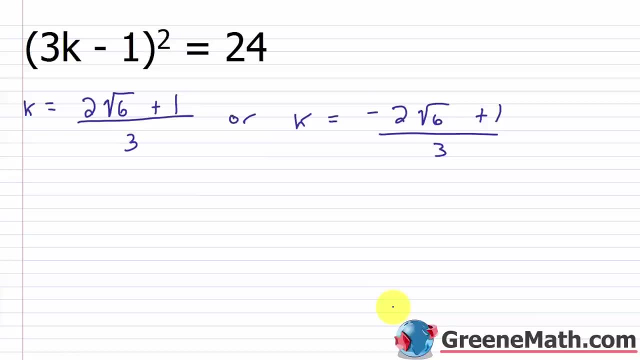 really, really tedious. so, because this is the last problem, we have some time. we're going to go back and check these two solutions, okay, so plugging this in will be kind of tedious. we're going to have an open parentheses. here we have three. and then times k is equal to 2 times the square root. 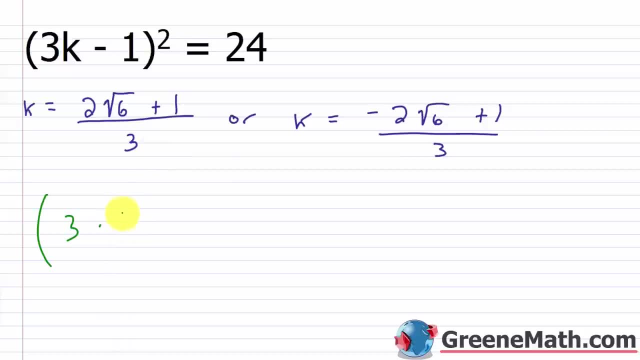 of k. so this is our value for k. so our value for k is 2 times the square root of 6, plus 1 over 3, and then we have minus 1, so then minus 1, this whole thing is squared and then it equals 24. 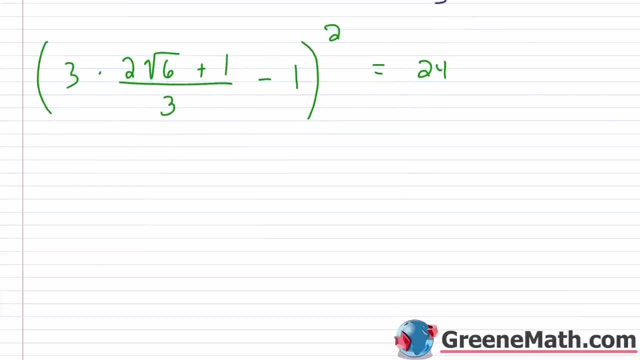 so, before I square anything, I want you to realize that you can cancel this 3 with this 3. so what would I have then inside? well, inside the parentheses now, I have 2 times the square root of 6 plus 1 minus 1. this is squared and it should equal 24. now these two would cancel, and I'm really. 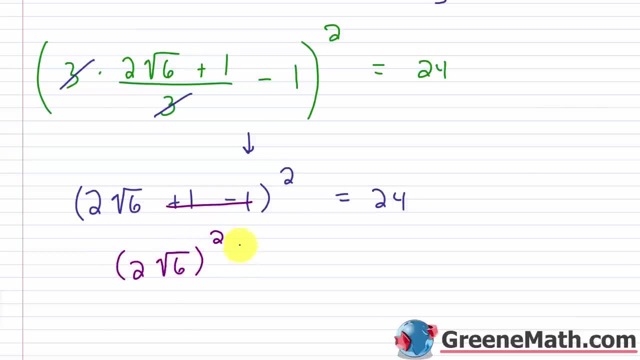 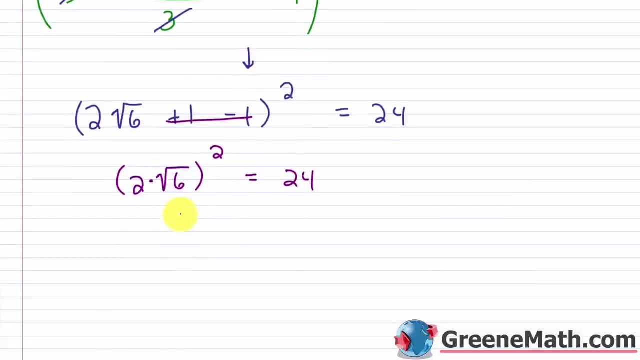 just left with 2 times the square root of 6. this is squared and it equals 24. let's keep scrolling down. now you realize that this is multiplication here. so really I have 2 squared times. the square root of 6 squared equals 24: 2 squared is 4. the square root of 6 squared equals 24. so I'm going to. 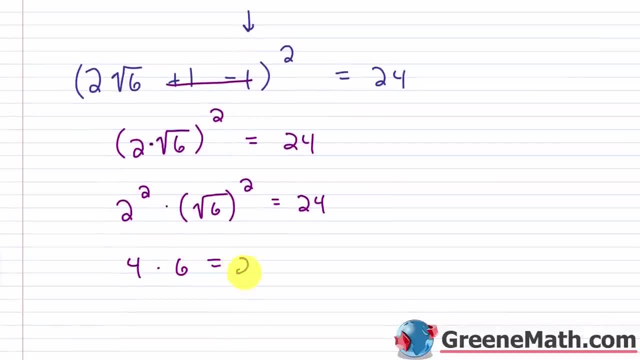 have 2 times the square root of 6. squared is 6, so 4 times 6 equals 24, and it does so. you get 24 equals 24, and again, this gets more and more tedious as you get higher in math. so I can't tell. 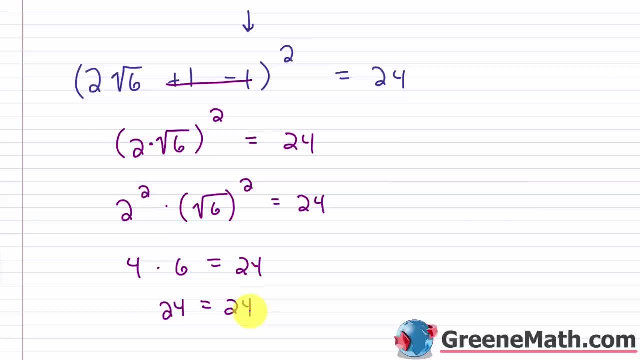 you that you're going to have time to check everything on your test, because in some situations you simply just won't have time. but you want to check as many things as you can, particularly if you go through your test and you finish everything up and you have time left. please take that time. 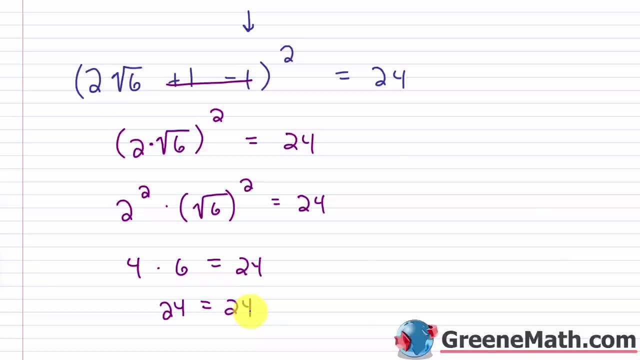 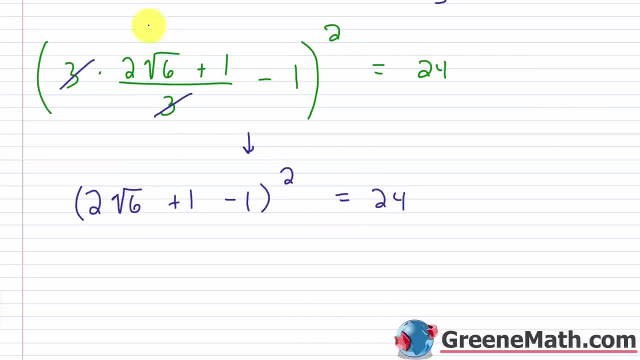 This is squared, and it should equal 24. Now, these two would cancel. And I'm really just left with 2 times the square root of 6. This is squared, and it equals 24. 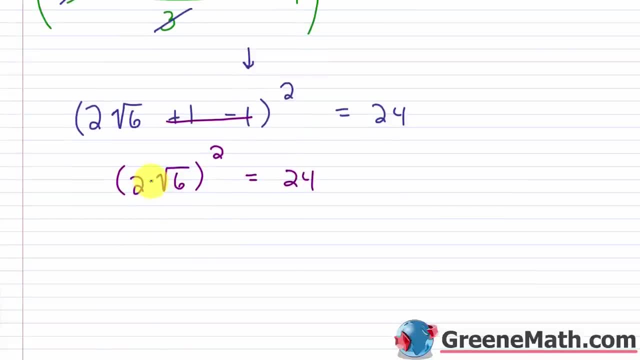 Let's keep scrolling down. Now, you realize that this is multiplication here. 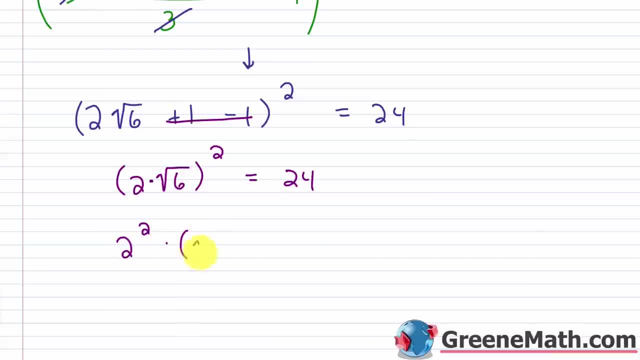 So really, I have 2 squared times the square root of 6 squared equals 24. 2 squared is 4. The square root of 6 squared is 6. 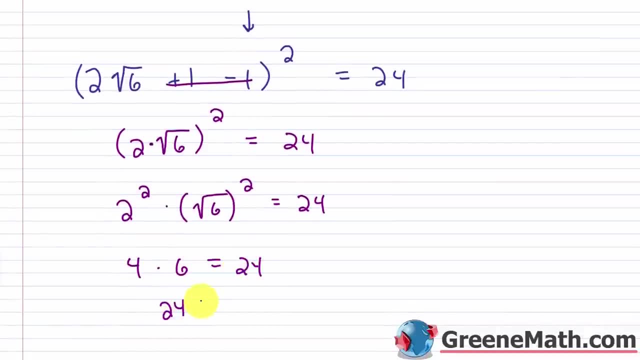 So 4 times 6 equals 24, and it does. So you get 24 equals 24. 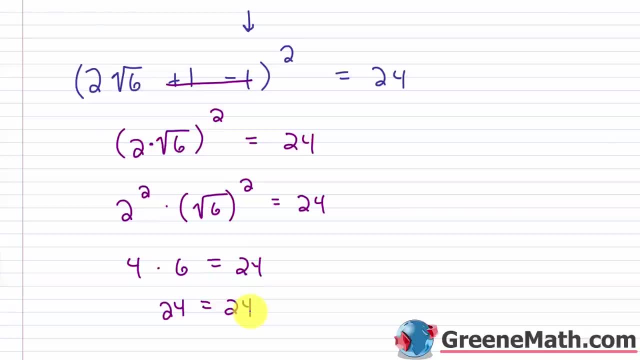 And again, this gets more and more tedious as you get higher in math. So I can't tell you that you're going to have time to check everything on your test, because in some situations, you simply just won't have time. 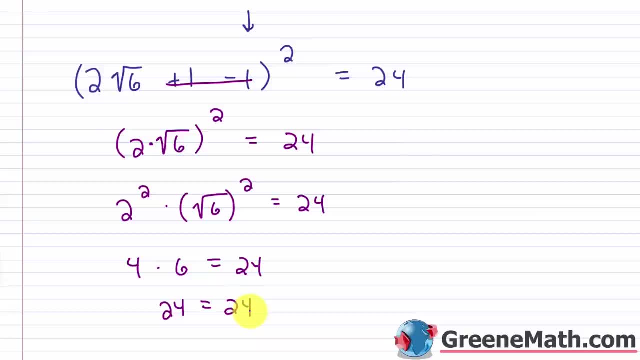 But you want to check as many things as you can, particularly if you go through your test, and you finish everything up, and you have time left, please take that time to go back and check as many answers as you can, because even if you catch one or two mistakes, that can save you from getting a B when you could have gotten an A. 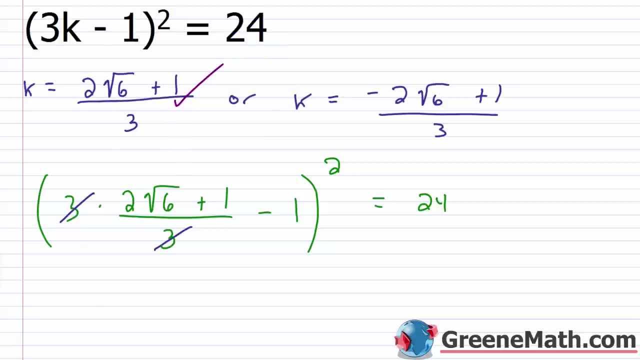 All right, so let's erase this. We'll put a checkmark here. And I'm going to reuse this, 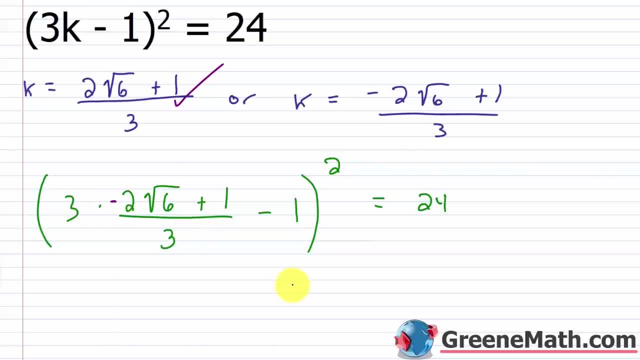 with the only exception of this being a negative out in front. 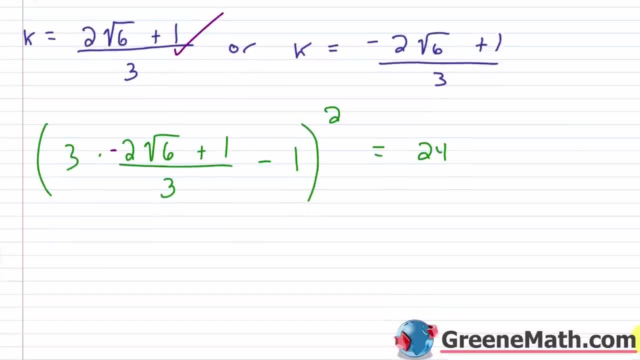 So the same thing is basically going to happen. Let me kind of scroll down a little bit. 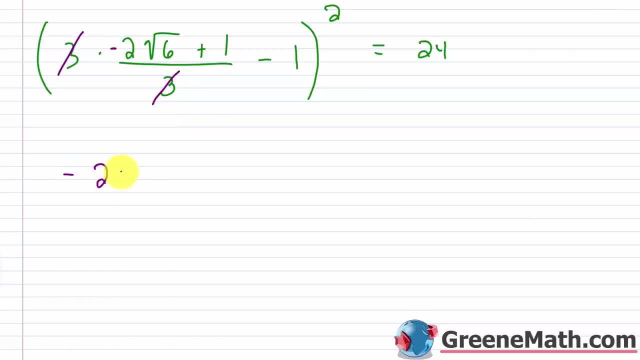 This again would cancel with this, and I'd have negative 2 times square root of 6 plus 1 minus 1. This would obviously cancel. So I have negative 2 times square root of 6. This is squared, and it equals 24. So now negative 2 is inside a parenthesis. So negative 2 would be squared, and then times square root of 6, which would be squared. 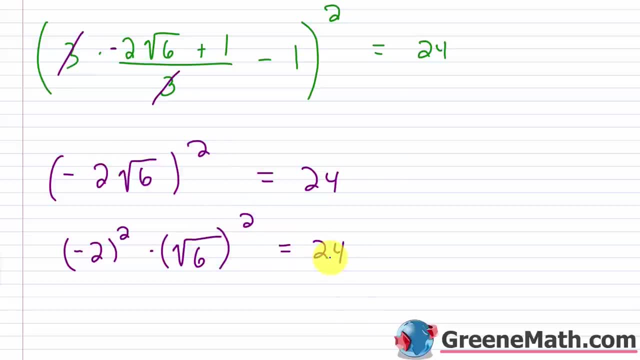 And I'm just using power to power rule here, equals 24. Negative 2 squared is 4, so you get 4 times square root of 6 squared is 6. This equals 24. And it does, you get 24 equals 24. 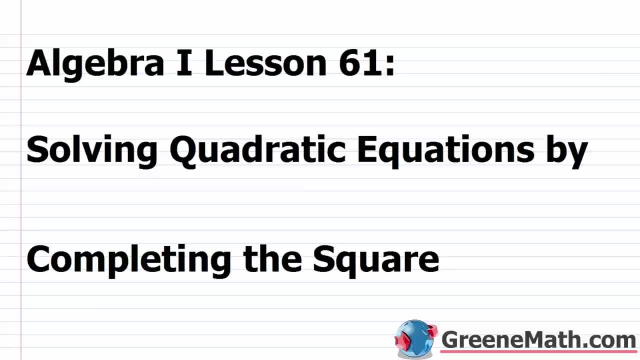 So this guy checks out as a valid solution as well. 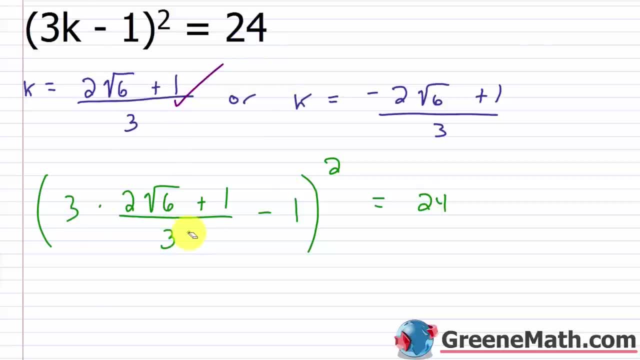 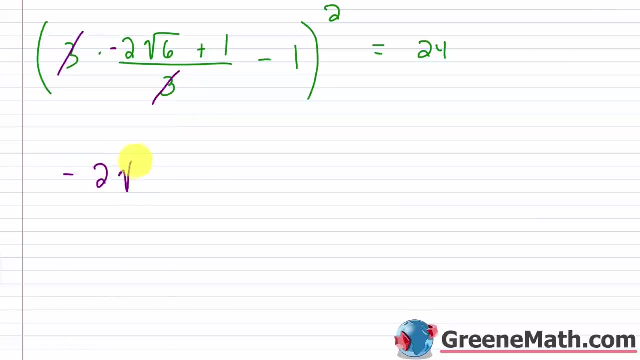 mark here and I'm going to reuse this, with the only exception of this being a negative out in front. so the same thing is basically going to happen. let me kind of scroll down a little bit. this again would cancel with this and I'd have negative 2 times square root of 6 squared. 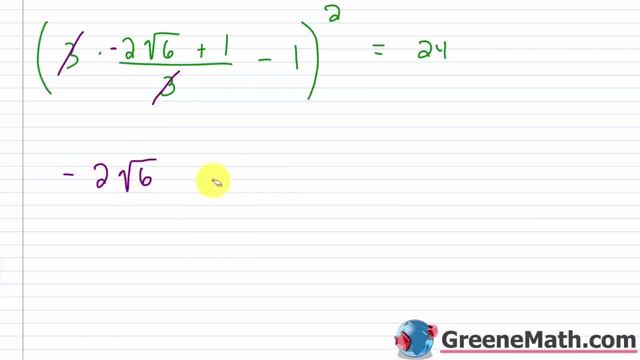 plus 1 minus 1. this would obviously cancel. so I have negative 2 times square root of 6. this is squared. it equals 24. so now negative 2 is inside a parentheses, so negative 2 would be squared. and then times square root of 6, which would be squared- and I'm just using power to power rule here- equals. 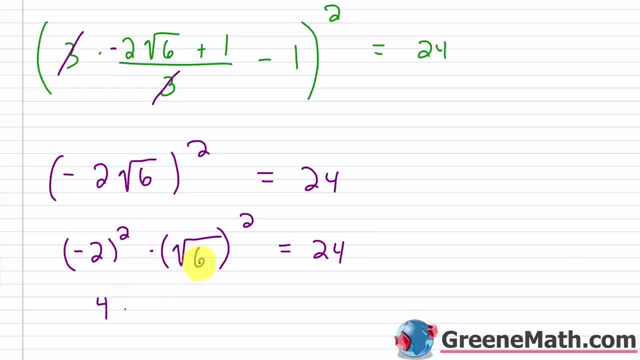 24 negative 2 squared is 4. so you get 4 times square root of 6, squared is 6. this equals 24, and it does you get 24 plus 1 minus 1. this is square root of 6. and then I'm going to do a little bit more. 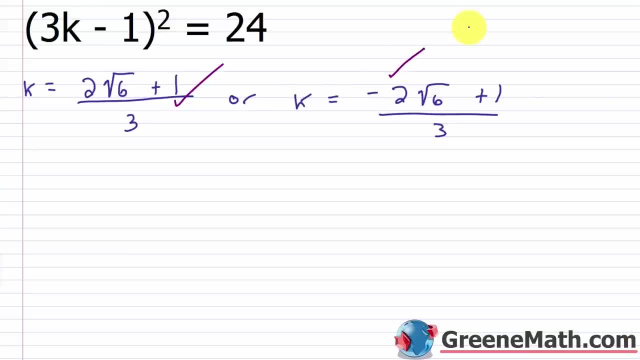 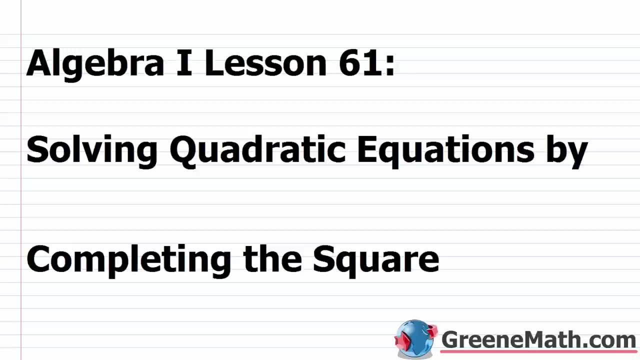 24 equals 24.. So this guy checks out as a valid solution as well. Hello and welcome to Algebra 1, Lesson 61.. In this video, we're gonna learn about solving quadratic equations by completing the square. So so far in this course. 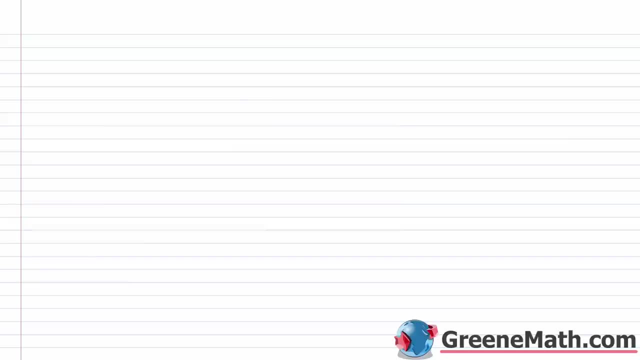 we've learned how to solve a quadratic equation by factoring, which we're not gonna be able to do in every scenario. And then also in the last lesson, we learned how to solve a quadratic equation by using something known as the square root property. 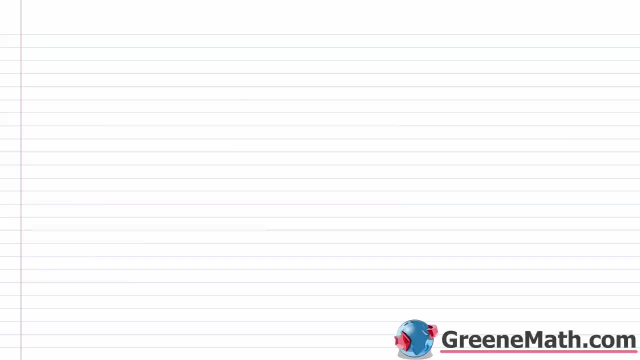 Now the thing about the square root property: you can use it on every quadratic equation, but you have to have the quadratic equation in a certain format to do that. So the purpose of this lesson is to learn how to complete the square, and that's gonna put it in a format. 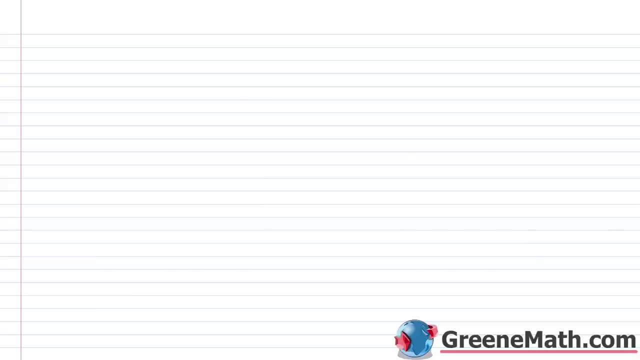 where you can use the square root property. So before we kind of jump in and start learning about this, I wanna make sure that everybody is on the same page with the square root, The square root property. So in the last lesson I started you off with something generic. 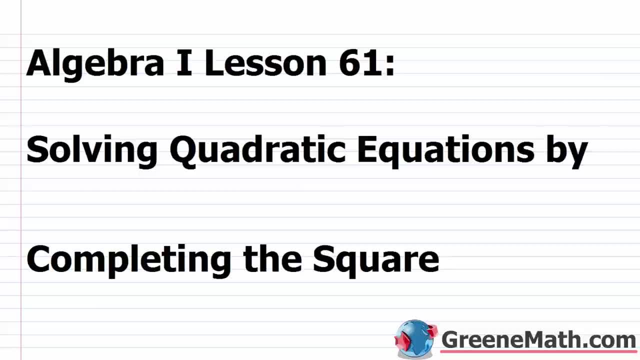 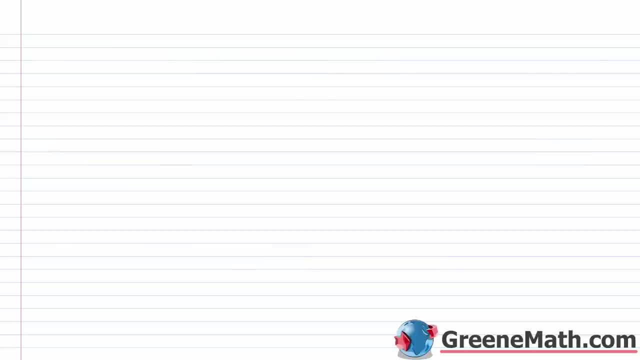 Hello, and welcome to Algebra 1 Lesson 61. In this video, we're going to learn about solving quadratic equations by completing the square. So, so far in this course, we've learned how to solve a quadratic equation by factoring, which we're not going to be able to do in every scenario. 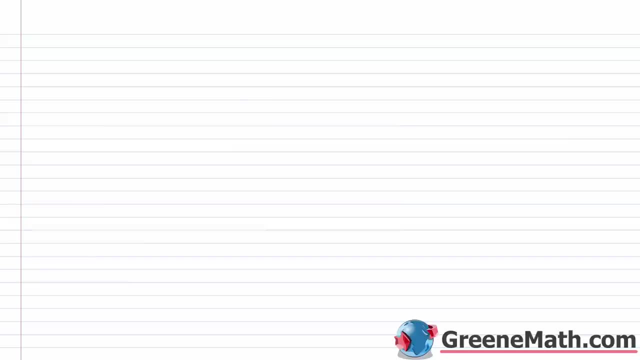 And then also in the last lesson, we learned how to solve a quadratic equation by using something known as the square root property. 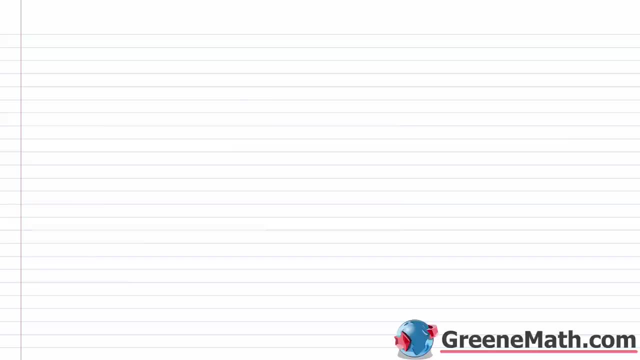 Now, the thing about the square root property, you can use it on every quadratic equation, but you have to have the quadratic equation in a certain format to do that. 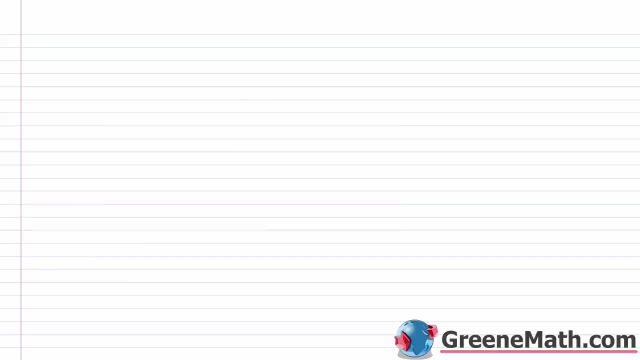 So the purpose of this lesson is to learn how to complete the square, and that's going to put it in a format where you can use the square root property. 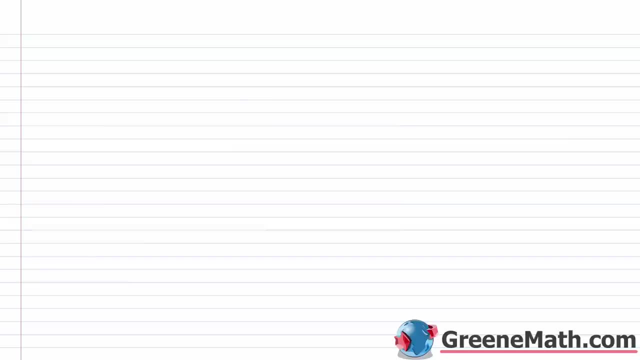 So before we kind of jump in and start learning about this, I want to make sure that everybody is on the same page with the square root property. 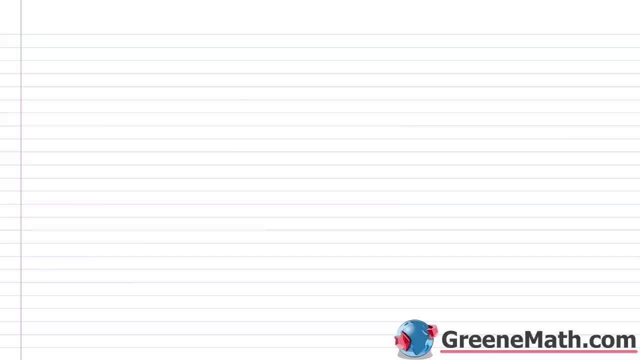 In the last lesson, I started you off with something generic, and I said if k was greater than zero, meaning k was positive, and we had something like x squared was equal to k, then what we said was that x could be equal to the principal square root of k, or x could be equal to the negative square root of k. 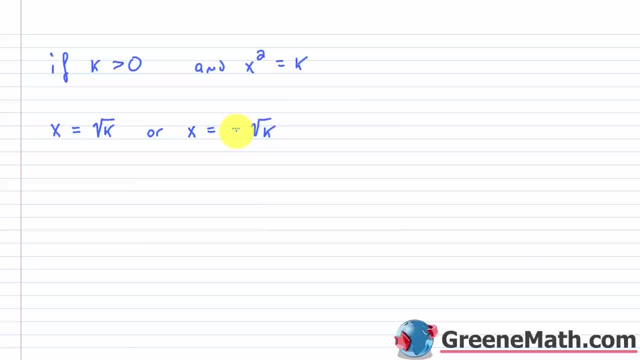 And it's important that you understand why we have these two solutions. 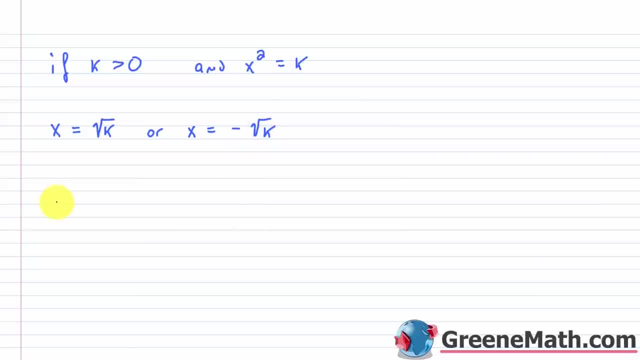 To use an example, let's say we saw something like x squared is equal to 64. Well, if I take the square root of this side right here, let me just rewrite this, that's going to undo the squaring. So I know that I will isolate x and have it by itself. But if I just take the principal square root of 64, that's not going to give me the whole picture. The principal square root of 64 by definition is 8. So x would equal 8 here. 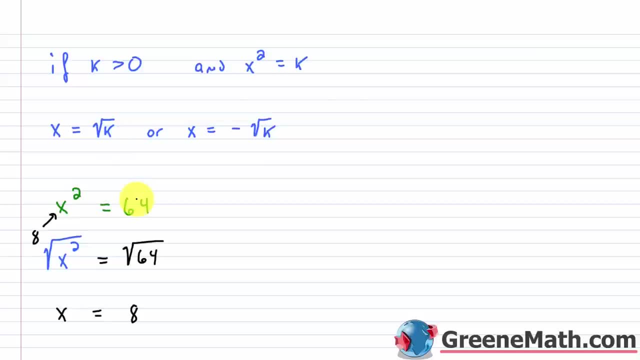 If I plugged in an 8 and I squared it, I would get 64. But just as it shows you here, 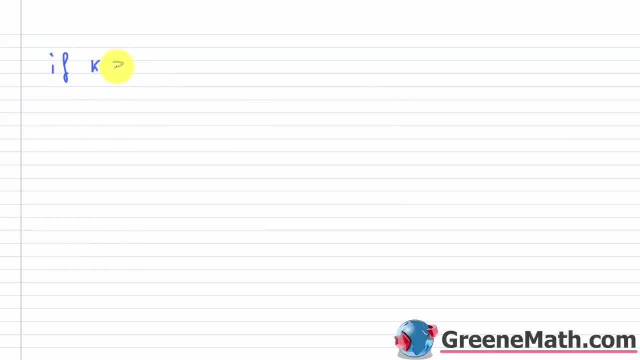 and I said if k was greater than zero, meaning k was positive, and we had something like x squared was equal to k, then what we said was that x could be equal to the principal square root of k or x could be equal to the negative square root of k. 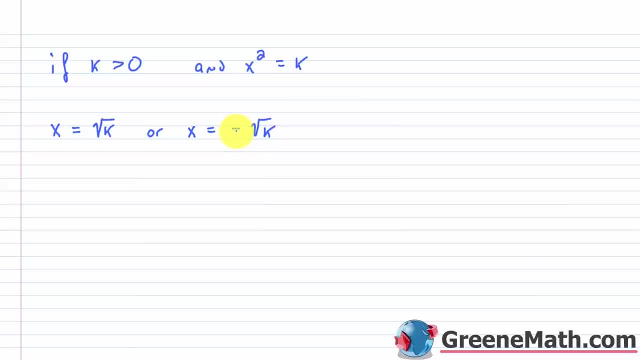 And it's important that you understand why we have these two solutions. To use an example, let's say we saw something like x squared is equal to 64.. Well, if I take the square root of this side right here, let me just rewrite this: 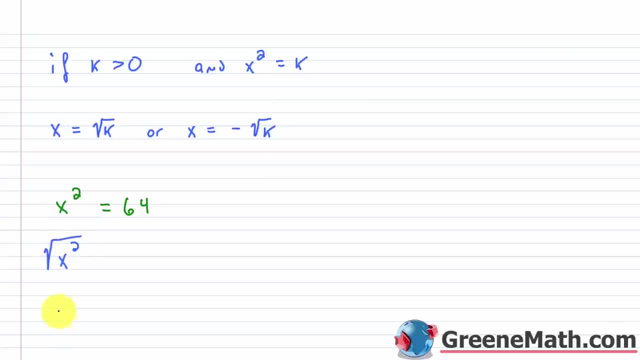 that's gonna undo the squaring. So I know that I will isolate x and have it by itself. But if I just take the principal square root of 64, that's not gonna give me the whole picture. The principal square root of 64,, by definition, is 64.64.. So I'm gonna take the principal square root of 64,. that's not gonna give me the whole picture. The principal square root of 64,, by definition, is 64.64.. So I'm gonna take the principal square root of 64, that's not gonna give me the whole picture. The principal square root of 64,, by definition, is 64.64.. 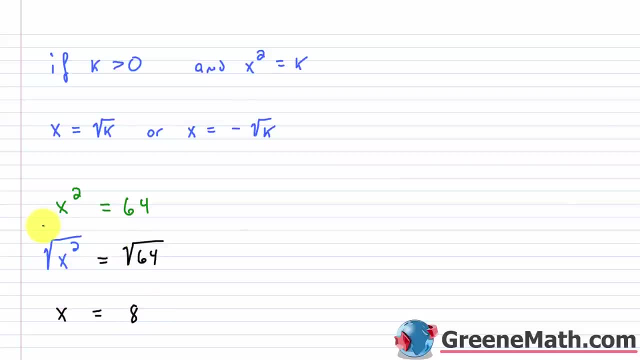 So x would equal eight. here, If I plugged in an eight and I squared it, I would get 64.. But just as it shows you, here I have the principal square root and the negative square root. So what I'd want here is a symbol. 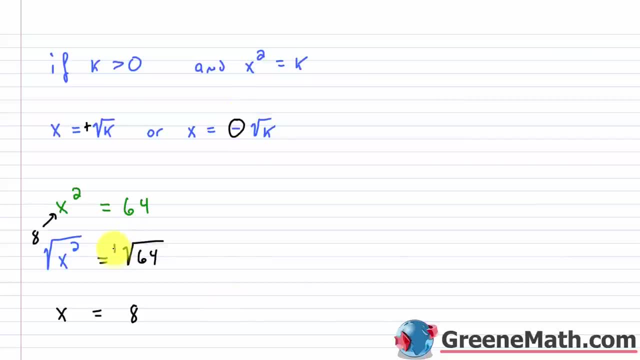 for the negative square root of 64 as well. So we put a plus and then a minus underneath, And this notation just tells me that I want the positive or principal square root of 64, along with the negative square root of 64.. 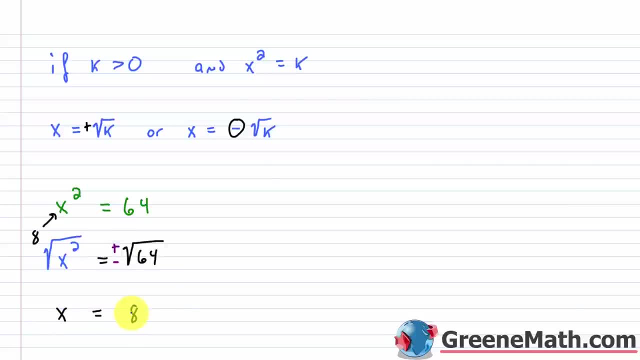 And so x would be eight, or x would also be the negative square root of 64, which is negative eight. And if I plugged in a negative eight for x, negative eight squared would also give me 64.. So this is just a way to account for both solutions. 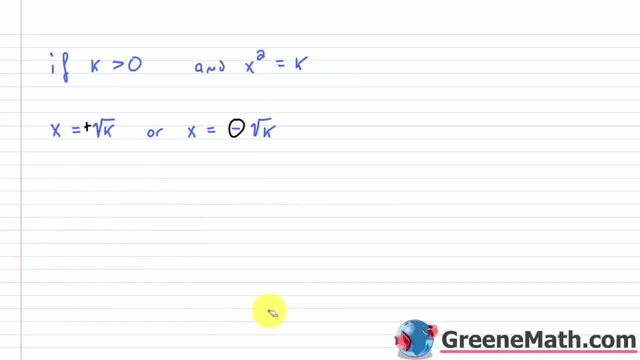 And if I use this on a more complex example, it's the same thing. Let's say I had something like the quantity x minus five, This is squared and it's equal to four. Now, if I take the square root of this side right here, 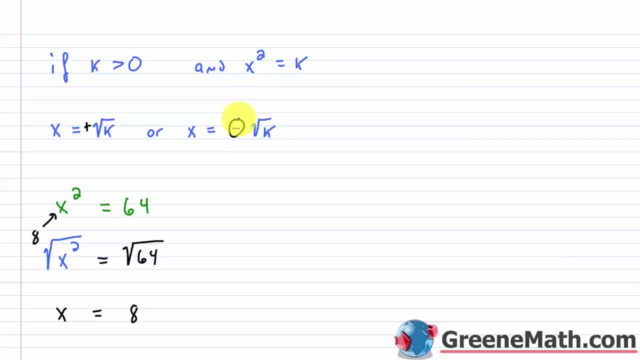 I have the principal square root and the negative square root. So what I'd want here is a symbol for the negative square root of 64 as well. So we put a plus and then a minus underneath. And this notation just tells me that I want the positive or principal square root of 64 along with the negative square root of 64. And so x would be 8. 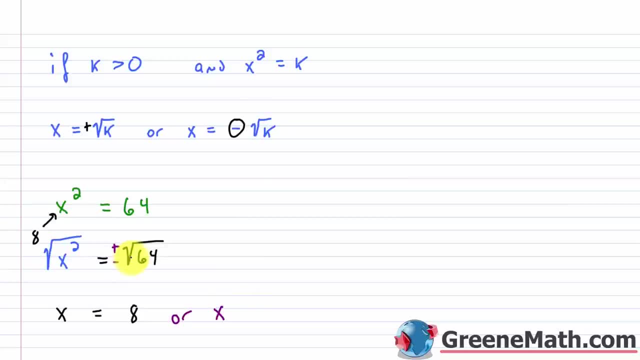 Or x would also be the negative square root of 64, which is negative 8. 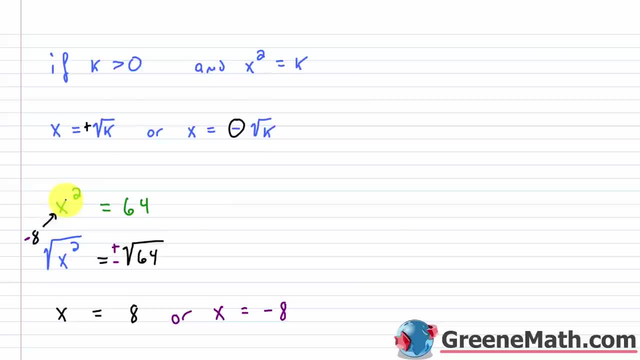 And if I plugged in a negative 8 for x, negative 8 squared would also give me 64. So this is just a way to account for both solutions. 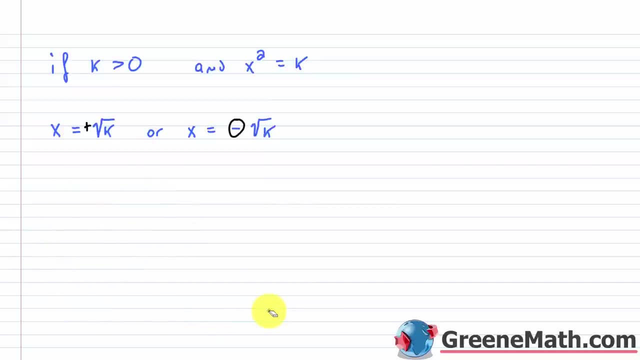 And if I use this on a more complex example, it's the same thing. 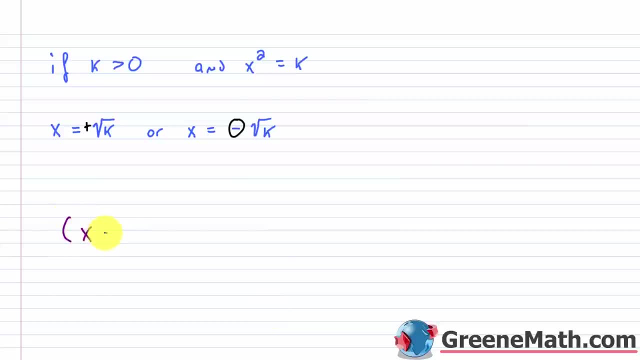 Let's say I had something like the quantity x minus 5. This is squared and it's equal to 4. Now, if I take the square root of this side right here, I would cancel this with the squared, right? So that's going to go away and I'm left with x minus 5. But over here, 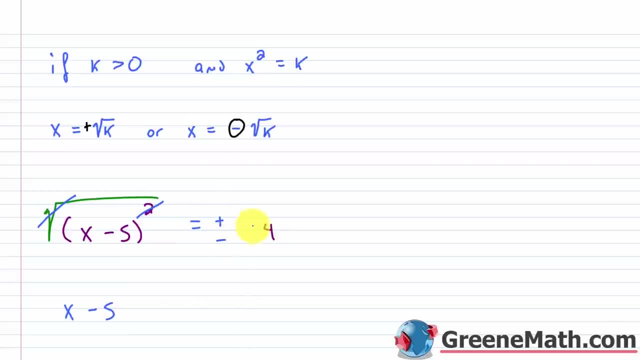 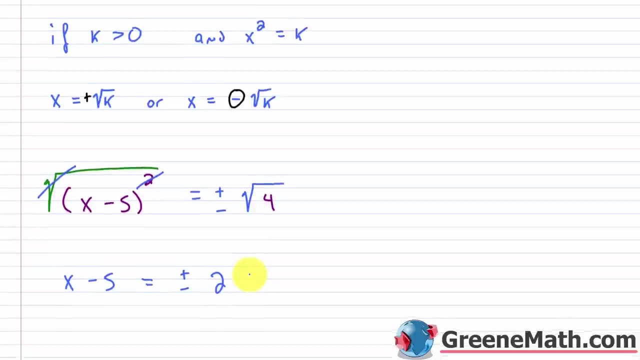 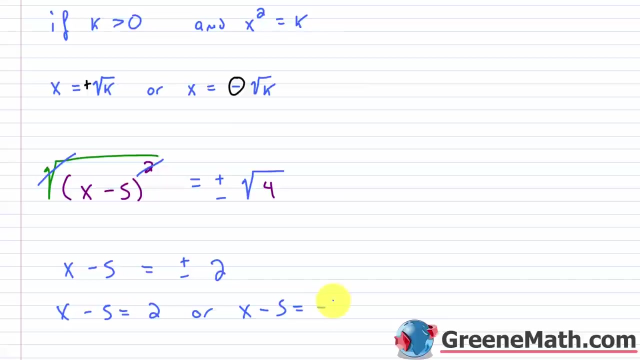 I've got to make sure that I account for the positive and the negative square root of 4. And when I solve this, I'm going to explain why. So let's say this is equal to... We know the square root of 4 is 2, so positive or negative 2, right? And you'd read that as plus or minus 2. So this is two different scenarios. It's x minus 5 is equal to 2 or x minus 5 is equal to negative 2. So let's pause for a minute and see why that would make sense, just without even doing anything else. Let me erase this. We're going to go back to the original equation. 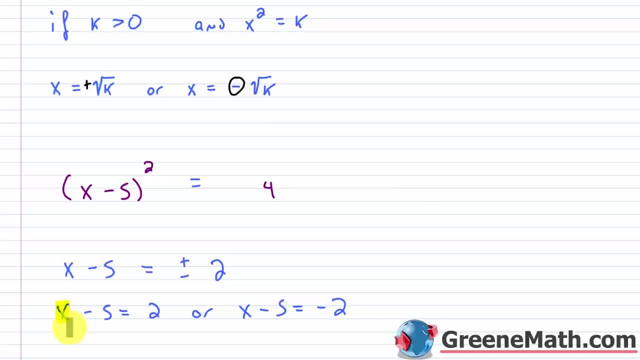 If you find a value for x that when plugged in, we subtract away 5 and get 2, well, that means that this value here would be 2. 2 squared. That would give me 4. Same thing over here. 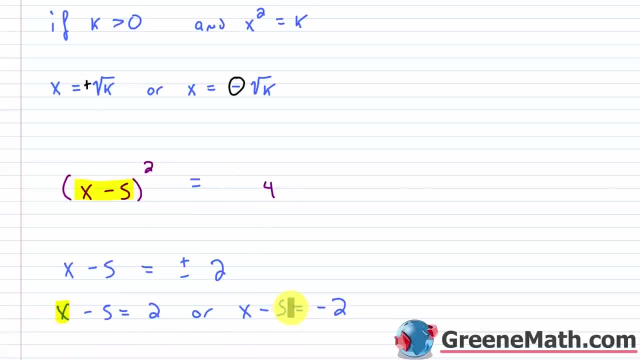 If I find a value for x that when plugged in, we subtract away 5, we get negative 2. Well, this in here would be negative 2. 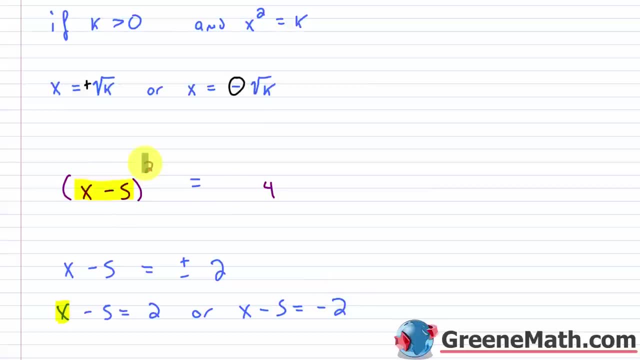 Negative 2 squared will also be 4. So we're accounting for those two possibilities. 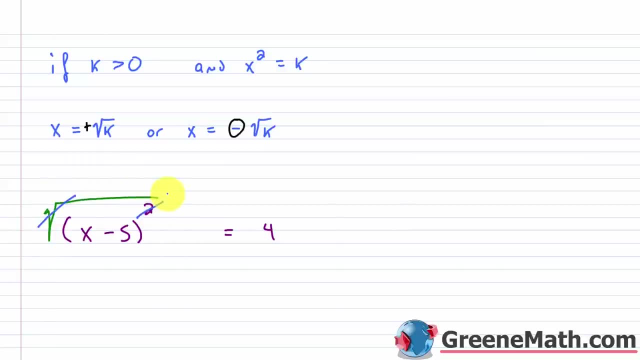 I would cancel this with the squared right. So that's gonna go away and I'm left with x minus five. But over here I've gotta make sure that I account for the positive and the negative square root of four, And when I solve this I'm gonna explain why. 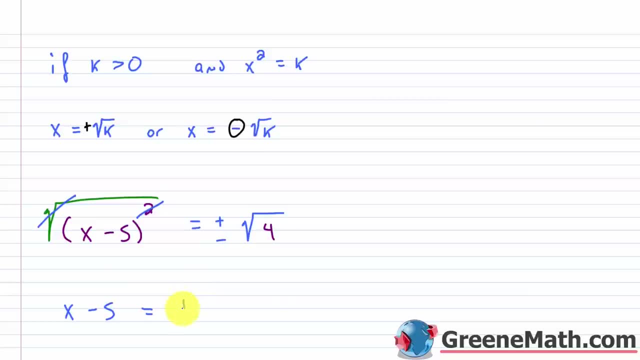 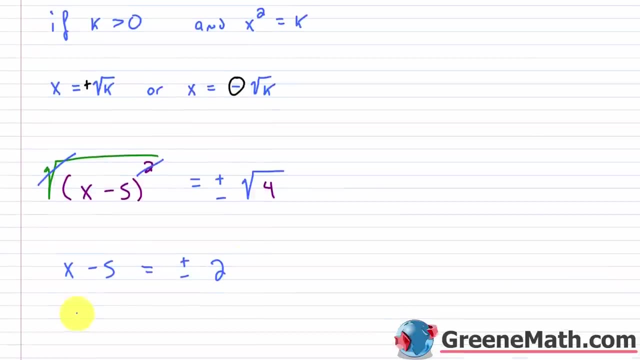 So let's say this is equal to. we know the square root of four is two. so positive or negative, two, right, We agree that is plus or minus two. So this is two different scenarios. It's x minus five is equal to two. 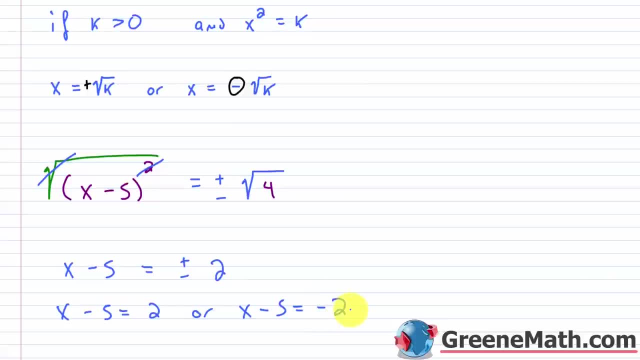 or x minus five is equal to negative two. So let's pause for a minute and see why that would make sense, just without even doing anything else. Let me erase this. We're gonna go back to the original equation. If you find a value for x that, when plugged in, 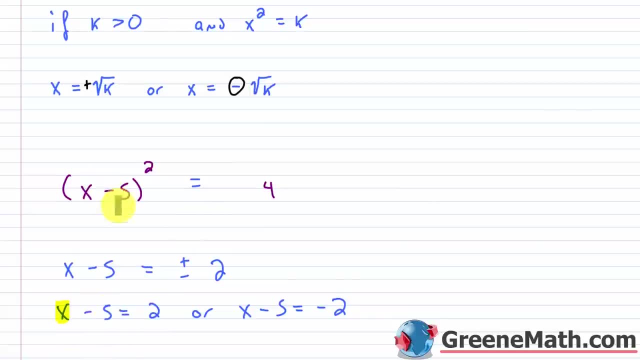 we subtract away five and get two. well, that means that this value here would be two. Two squared would give me four. Same thing over here. If I find a value for x that, when plugged in we subtract away five, we'll get negative two. 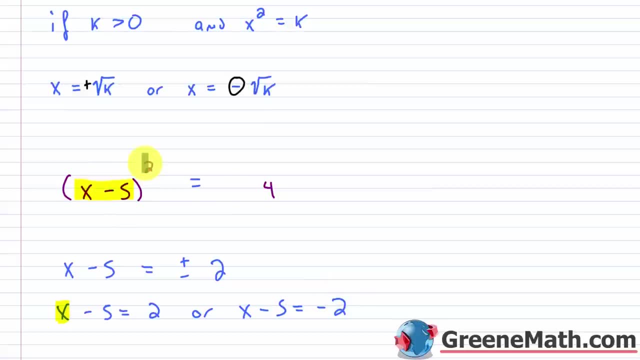 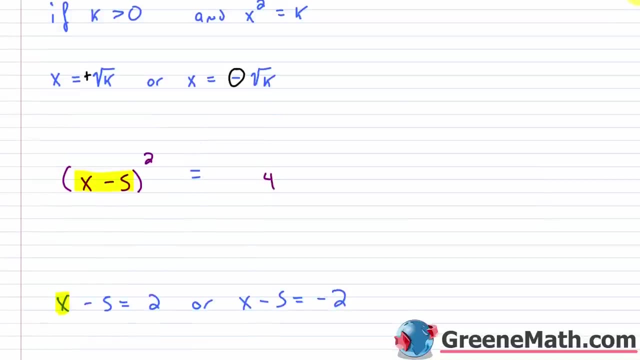 Well, this in here would be negative two, Negative two. squared will also be four. So we're accounting for those two possibilities. So let me just erase this real quick And we're gonna solve this and I'm gonna show you that. 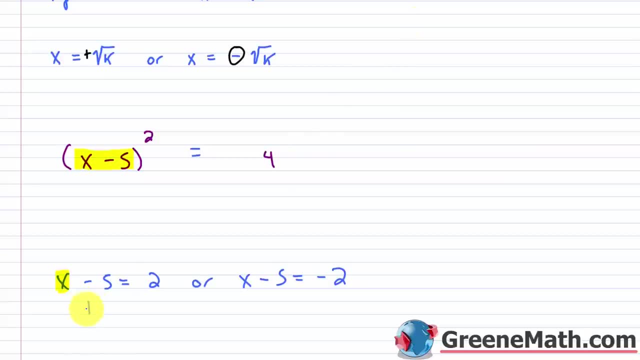 So if I add five, if I add five to both sides of the equation, I'd get x is equal to seven. If I add five to both sides of the equation here, I would get x is equal to three. Plug in a seven there. 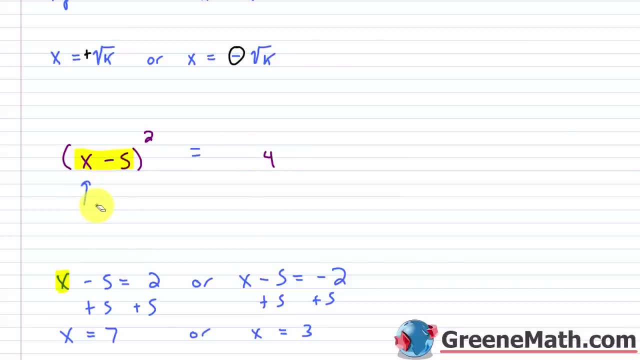 Seven minus five is two. Two squared is four. Plug in a three there. Three minus five is negative two, The negative two. and just to show you this, the negative two would be inside of parentheses. Negative two squared would also be four. 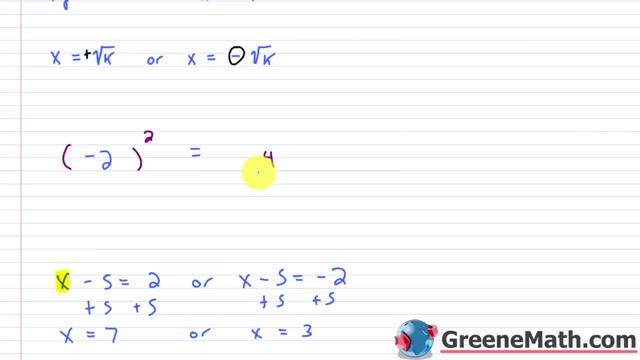 So that's why it's so important to make sure we put that plus or minus out in front. as we've shown here, We could write this as: x is equal to, plus or minus, the square root of k, So now that we've reviewed the square root property, 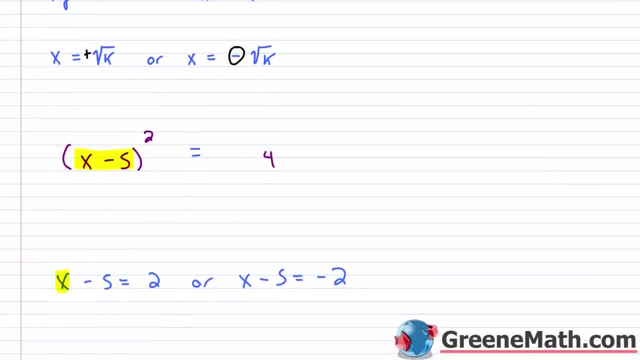 And we're going to solve this and I'm going to show you that. So if I add 5, if I add 5 to both sides of the equation, I get x is equal to 7. 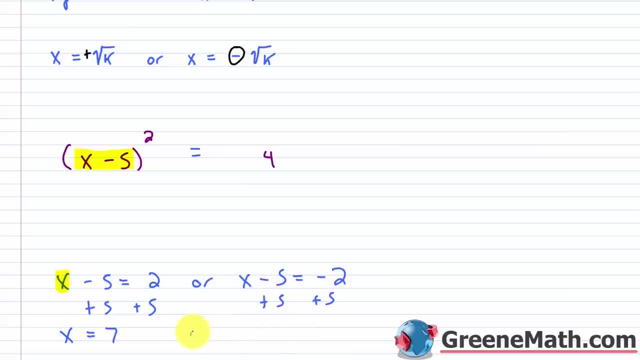 If I add 5 to both sides of the equation here, I would get x is equal to 3. 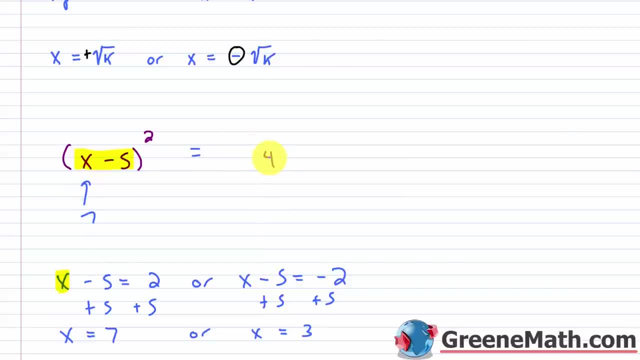 Plug in a 7 there. 7 minus 5 is 2. 2 squared is 4. 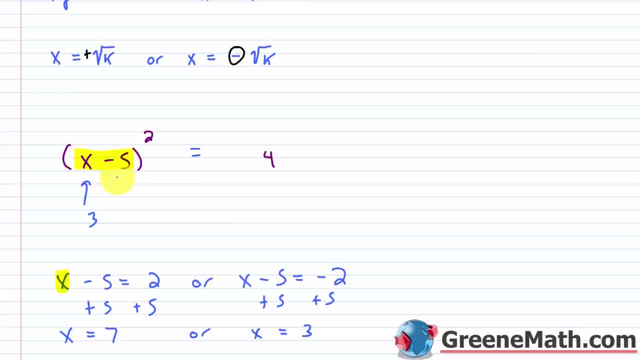 Plug in a 3 there. 3 minus 5 is negative 2. The negative 2, and just to show you this, the negative 2 would be inside of parentheses. 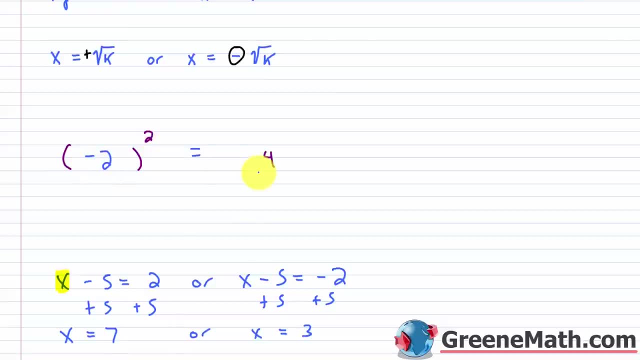 Negative 2 squared would also be 4. So that's why it's so important to make sure we put that plus or minus out in front, as we've shown here. 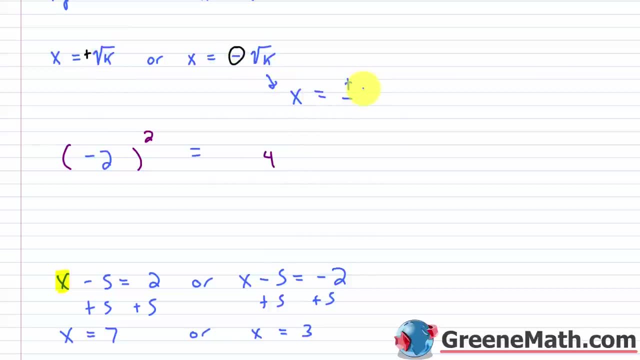 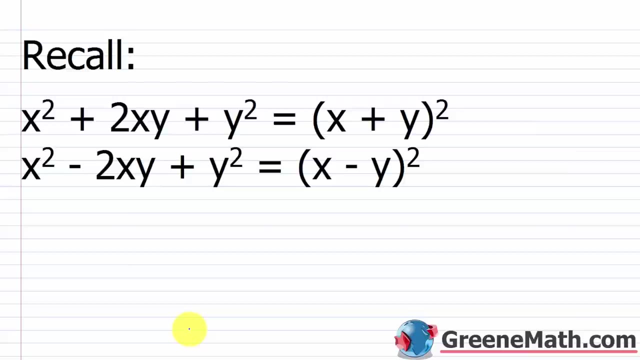 And we could write this as x is equal to plus or minus the square root of k. So now that we've reviewed the square root property, I want to just take a minute and talk about a perfect square trinomial. 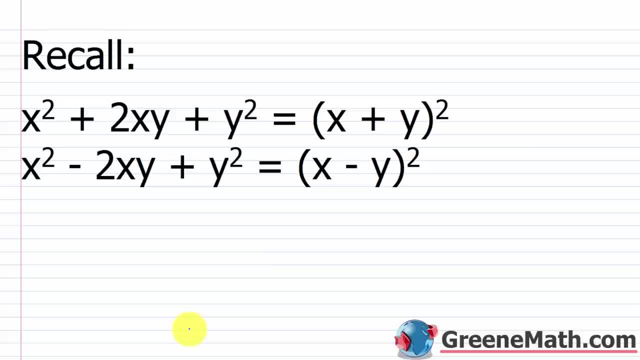 So before we get to that, remember, a perfect square in general is just a number with a rational square root. So something like 4, or let's say 100, or 169. 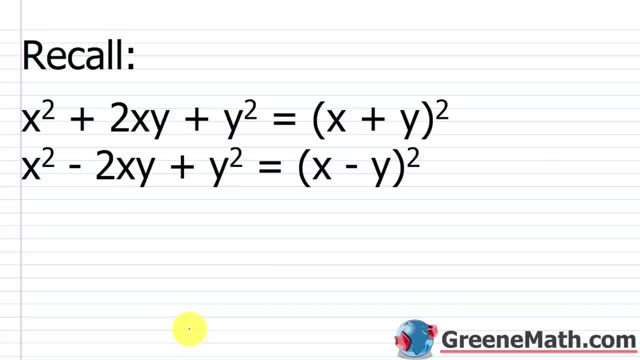 If I take the square root of that number, I'm going to get a rational number back. So... Something like 4, if I take the square root, I get 2. Something like 100, if I take the square root, I get 10. Something like 169, if I take the square root, I get 13. But something that's not a perfect square, let's say I take the square root of 5. 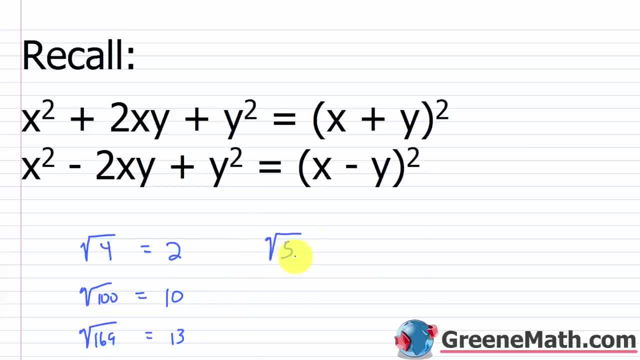 Square root of 5. Well, we know that this is an irrational number. And if we were to try to write this out in decimal form, the decimal does not terminate, and it does not repeat the same pattern forever and ever and ever. 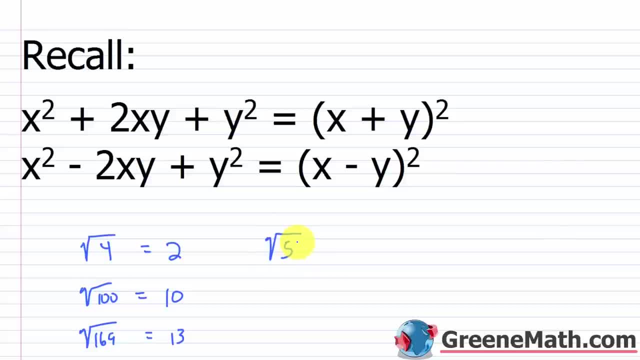 So we end up having to approximate these. So that's the difference between having something that's a perfect square and not a perfect square. When we get more advanced into this, we talk about something known as a perfect square trinomial. 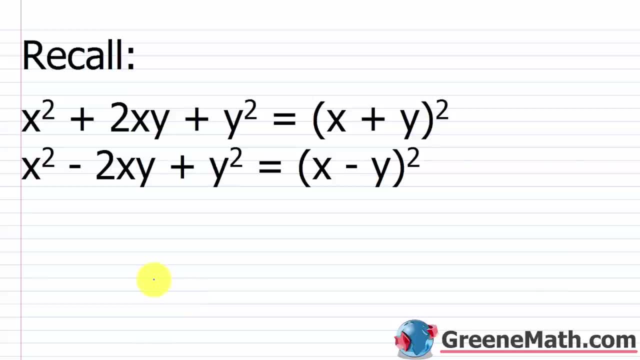 And I gave you this back when we talked about special products, back when we talked about special factoring. But you might not have understood what it was yet because we hadn't really developed everything. 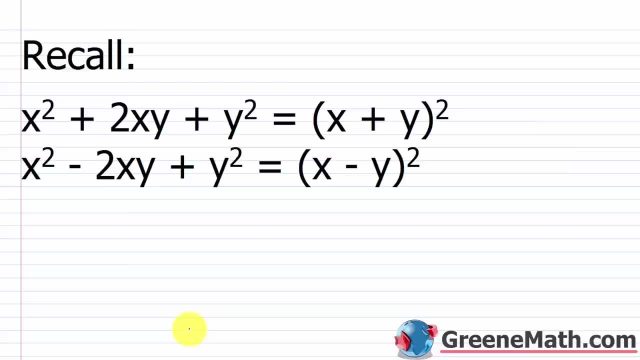 wanna just take a minute and talk about a perfect square, trinomial. So before we get to that, remember a perfect square in general is just a number with a rational square root, So something like four or let's say 100, or 169.. 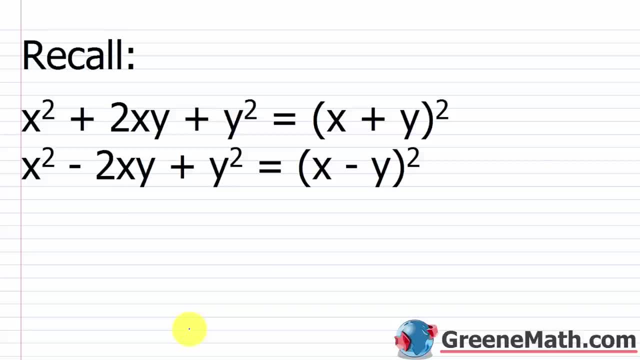 If I take the square root of that number, I'm gonna get a rational number. I'm gonna get a rational number back. So something like four. if I take the square root, I get two, Something like 100,. if I take the square root, I get 10.. 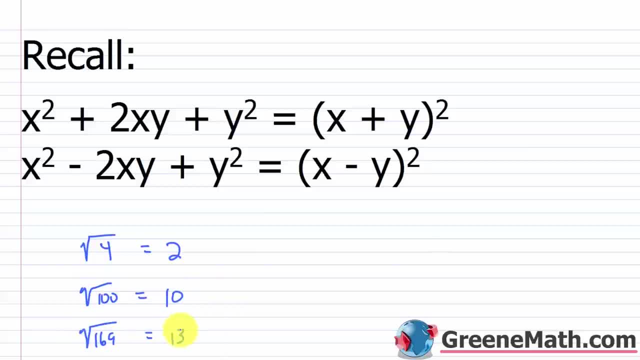 Something like 169,. if I take the square root, I get 13.. But something that's not a perfect square. let's say, I take the square root of five, Square root of five. Well, we know that this is an irrational number. 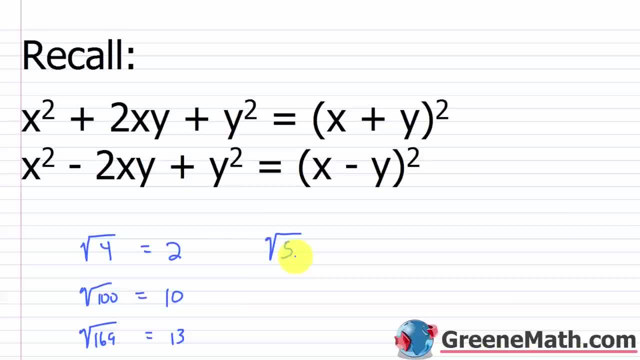 and if we were to try to write this out in decimal form? the decimal does not terminate and it does not repeat the same pattern forever and ever and ever. So we end up having to approximate these. So that's the difference between having something. 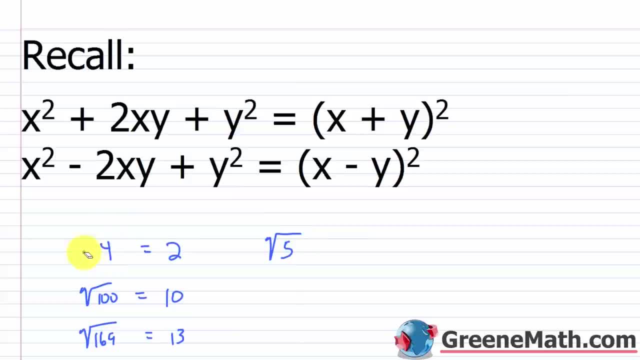 that's a perfect square and not a perfect square. When we get more advanced into this, we talk about something known as a perfect square, trinomial, And I gave you this back when we talked about special products, back when we talked about special factoring. 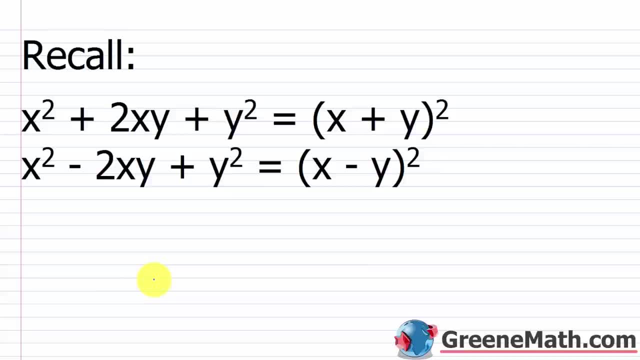 but you might not have understood what it was yet because we hadn't really developed everything. Now you should have a complete understanding of what a perfect square trinomial is. A perfect square trinomial is just a trinomial that can be factored as the square of a binomial. 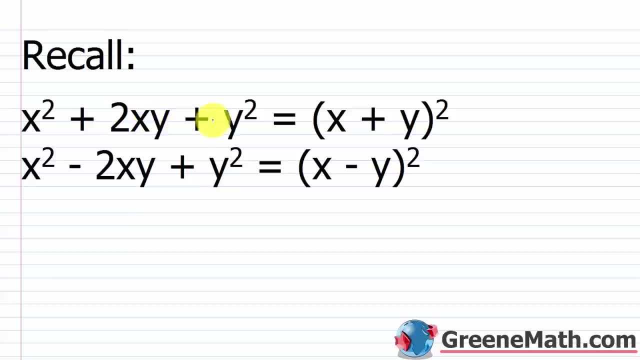 So, as an example, x squared plus two xy plus y squared can be factored as the square of a binomial. X squared minus two xy plus y squared can be factored as the square of a binomial, Something like x squared plus 10x. 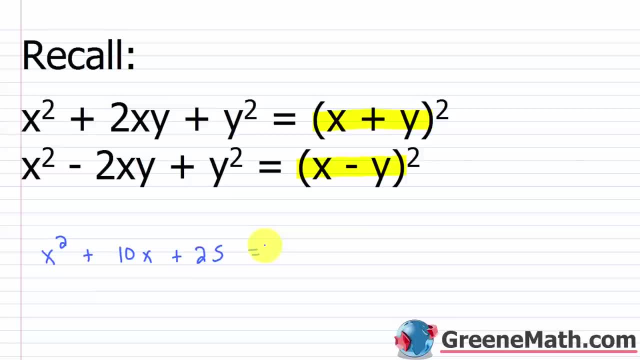 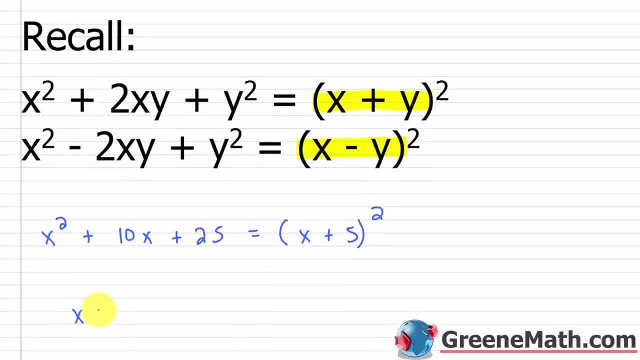 plus 25 can be factored into x plus 5, that quantity squared. Now, why would something like this be important for us in this lesson? Well, remember, I just showed you that if you have something in this format, let's say, I had x plus 5, that quantity squared, and it was equal. 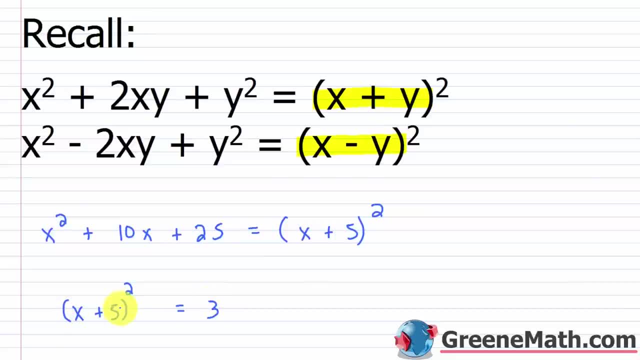 to some number. Let's just say it's equal to 3.. Well, I know I can solve this using the square root property. So what we're going to be doing in this lesson is we're going to take trinomials. 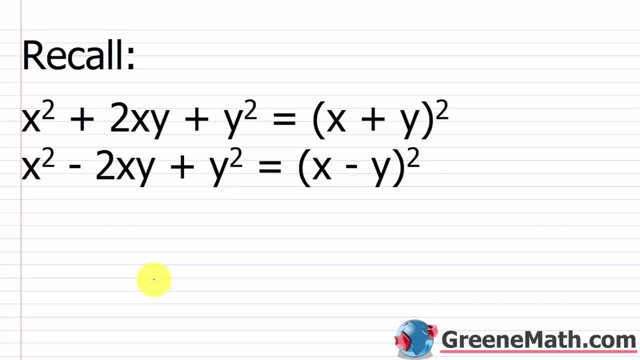 Now you should have a complete understanding of what a perfect square trinomial is. A perfect square trinomial is just a trinomial that can be factored as the square of a binomial. 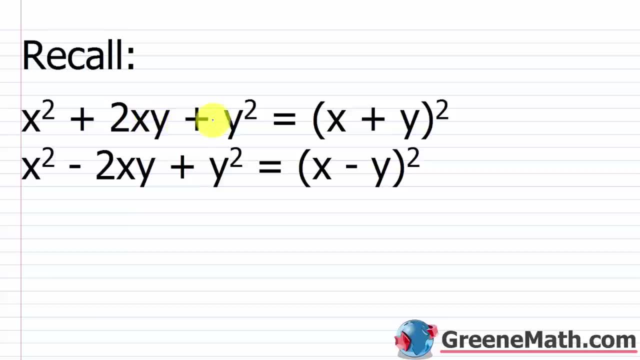 So as an example, x squared plus 2xy plus y squared can be factored as the square of a binomial. x squared minus 2xy plus y squared can be factored as the square of a binomial. Something like x squared plus 10x plus 25. Can be factored into x plus 5 that quantity squared. 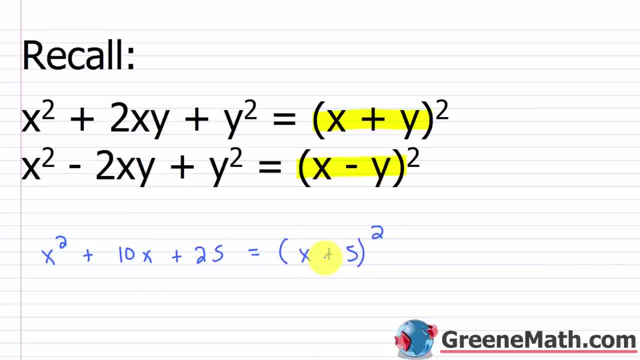 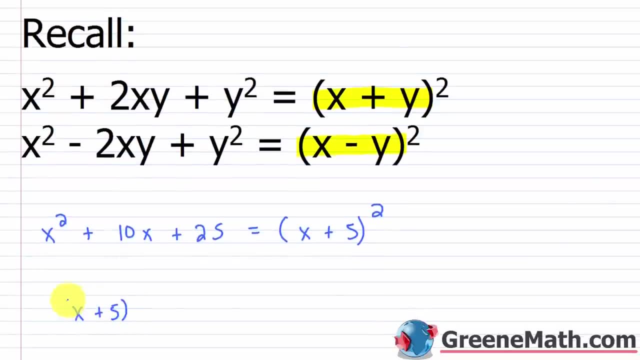 Now why would something like this be important for us in this lesson? Well remember I just showed you that if you have something in this format, let's say I had x plus 5 that quantity squared and it was equal to some number. Let's just say it's equal to 3. 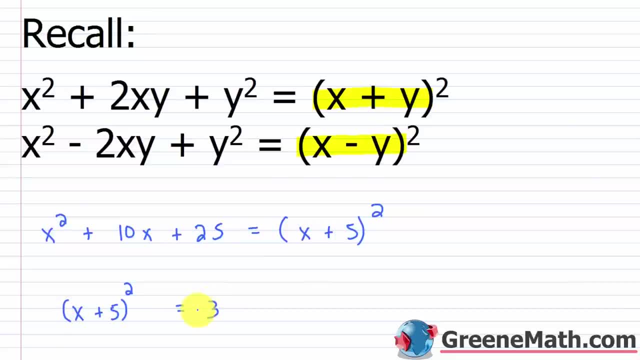 Well I know I can solve this using the square root property. So what we're going to be doing in this lesson is we're going to create trinomials that are not perfect square trinomials and we're going to make them into perfect square trinomials through a process known as completing the square. Okay, so you're going to see we're going to do that and then we're going to get the left side into this format, the right side as just a number or a constant, and then we're going to use the square root property to end up getting our solution. 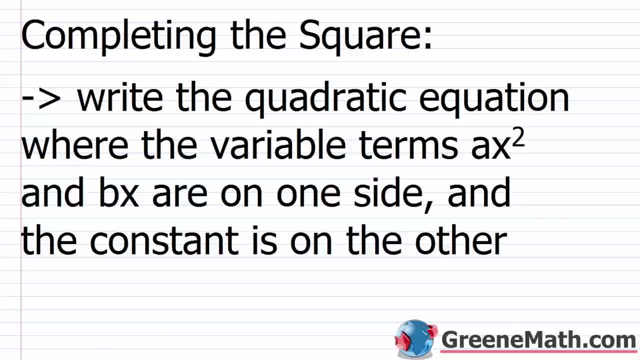 Alright, so here's the official procedure for completing the square. 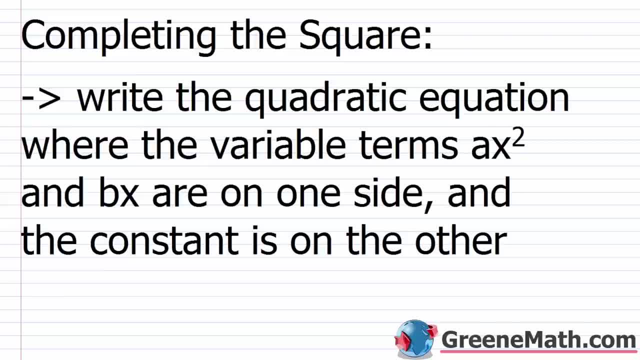 And I would advise you to write this down and use it as we work through these problems. 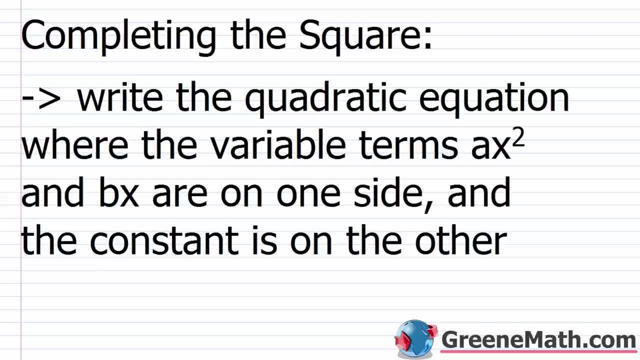 And then in your textbook I would just refer to this sheet over and over and over again until you are just flowing through these problems and you've memorized this process. 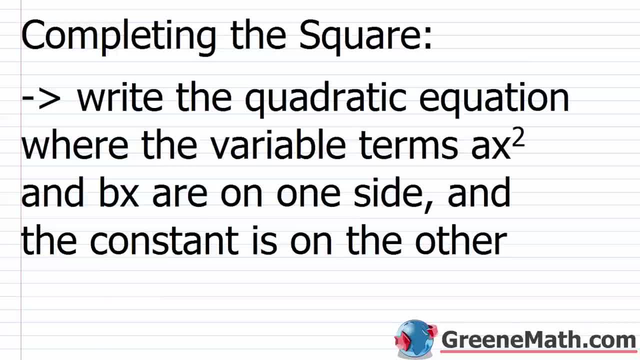 So you want to write the quadratic equation where the variable terms, okay, the variable terms ax squared and bx are on one side and the constant is on the other. So all the terms with variables on one side, all the constants on the other. 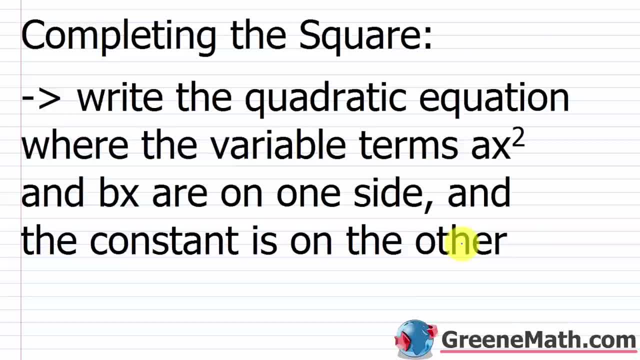 And you're just going to use the addition property of equality to move things around. 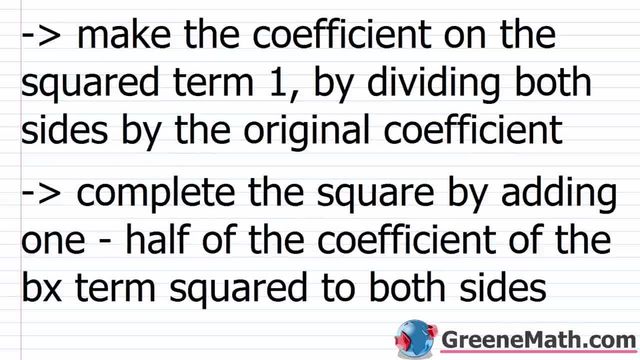 Now, the next thing you want to do, and this may or may not be necessary, depends on what kind of problem you're looking at. 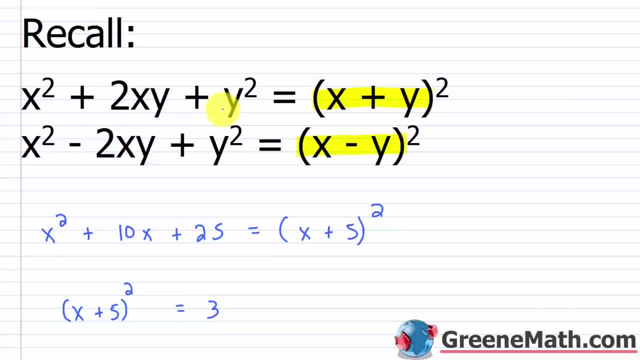 that are not perfect square trinomials, and we're going to make them into perfect square trinomials through a process known as completing the square. okay, So you're going to see, we're going to do that, and then we're going to get the left side into this format, the right side as just a number. 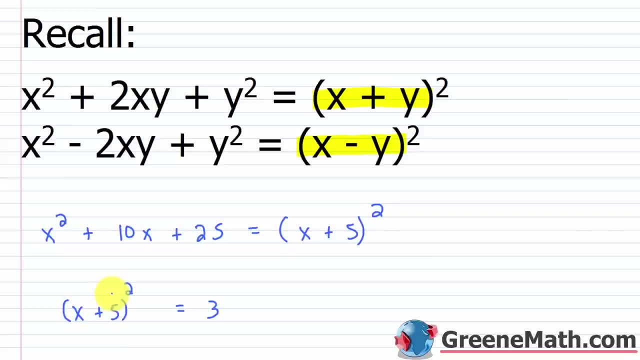 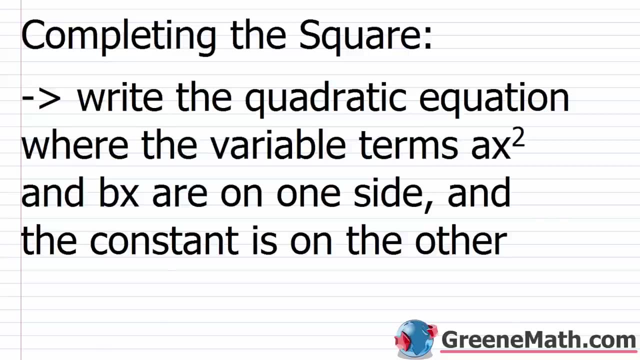 or a constant, and then we're going to use the square root property to end up getting our solution All right. So here's the official procedure for completing the square, And I would advise you to write this down and use it as we work through these problems And then in your 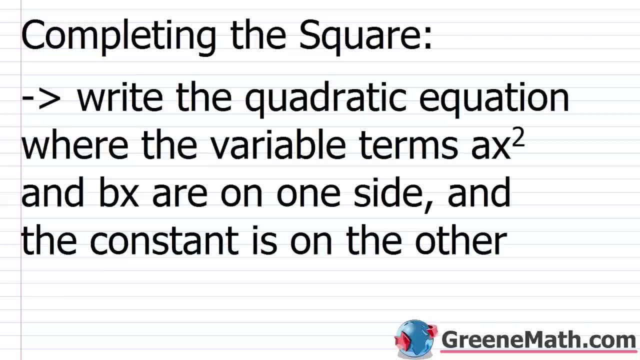 textbook. I would just refer to this sheet over and over and over again until you are just flowing through these problems and you've memorized this process. So you want to write the quadratic equation where the variable terms- okay, the variable terms- ax, squared and bx are on one side. 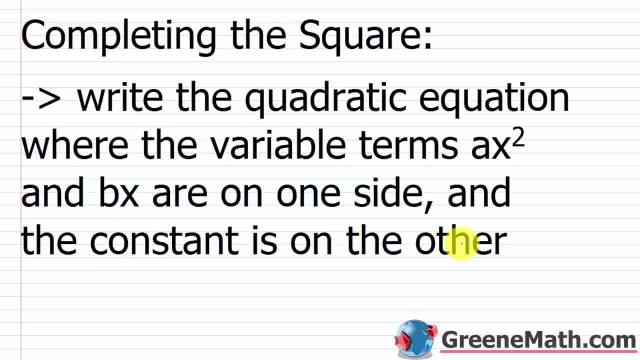 and the constant is on the other side. So you're going to write this down and you're going to on the other. So all the terms with variables on one side, all the constants on the other, And you're just going to use the addition property of equality to move things around. 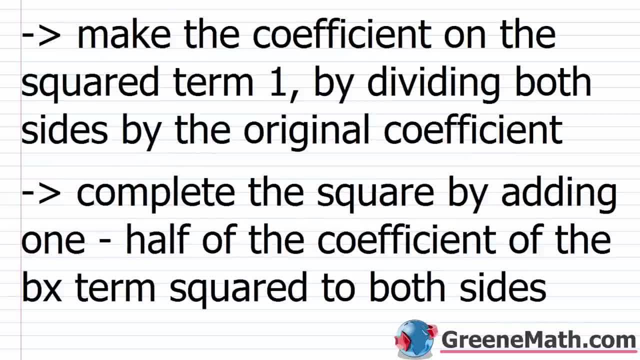 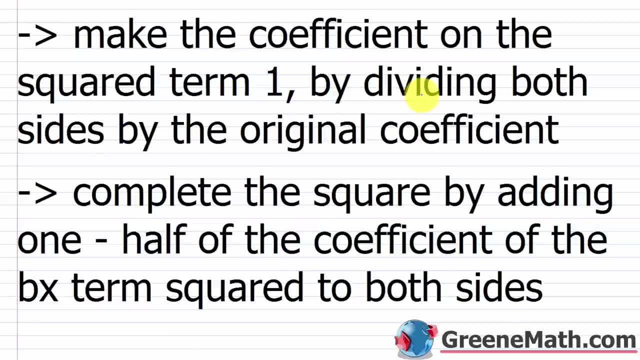 Now the next thing you want to do- and this may or may not be necessary depends on what kind of problem you're looking at- you want to make the coefficient on the squared term one by dividing both sides by the original coefficient In the beginning of your textbook. 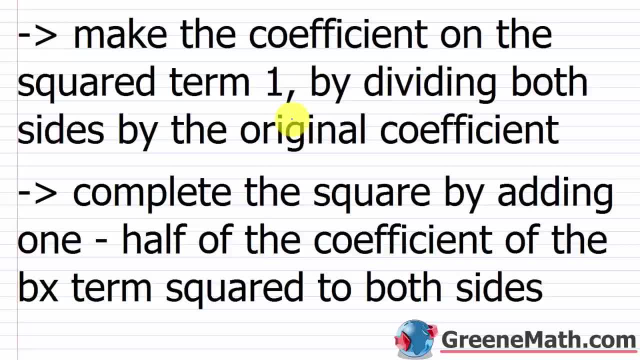 the problems they're going to give you will be easy and you won't have to do this. You'll just have an x squared, But later on you'll get something like 6x squared or 10x squared or 9x squared where you're going to have to deal with that. But you want the coefficient. 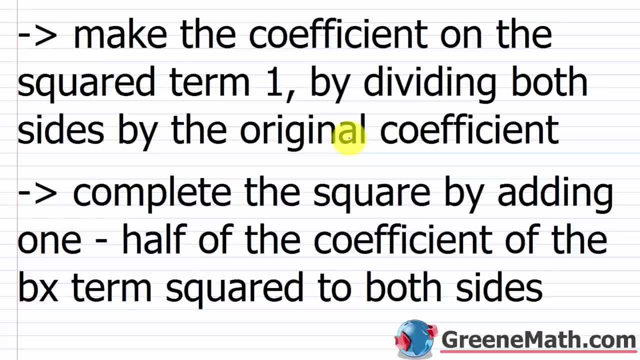 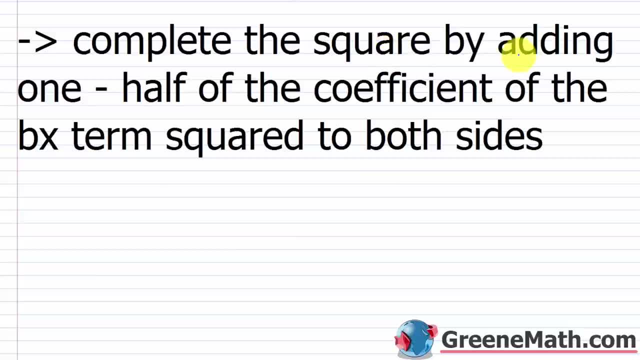 on the squared term to be one. Alright. so here comes the next step, and this is the one that everybody gets wrong when they first start out. You're going to complete the square by adding one half of the coefficient of the bx term, squared to both sides. 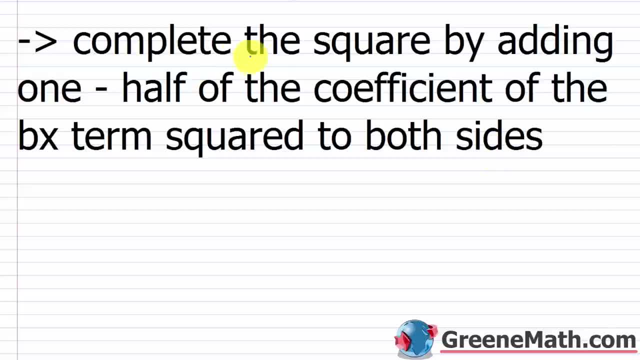 Okay, let me just re-read that: Complete the square by adding one half of the coefficient of the bx term, squared to both sides. So I want you to write in your notes: cut it in half, then square it. This is how my eighth grade teacher taught it to me, and it's stuck. 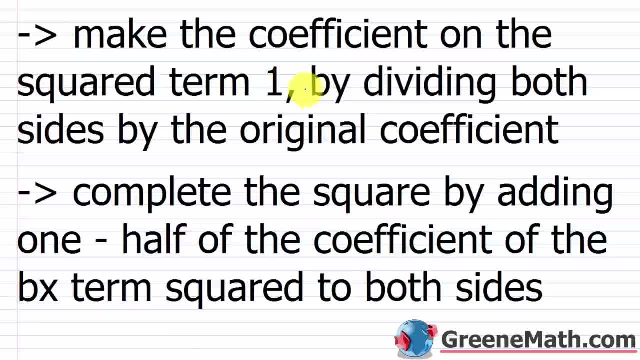 You want to make the coefficient on the squared term one by dividing both sides by the original coefficient. 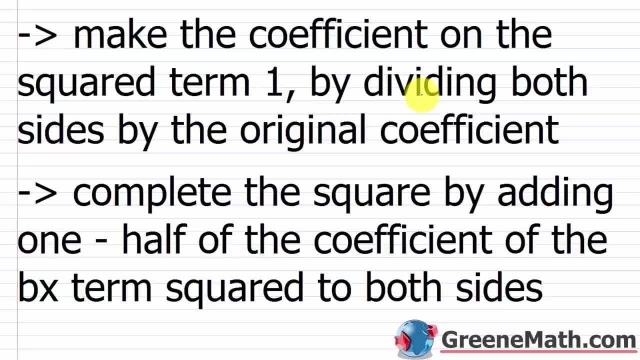 In the beginning of your textbook, the problems they're going to give you will be easy and you won't have to do this. Right, you'll just have an x squared. But later on, you'll get something like, 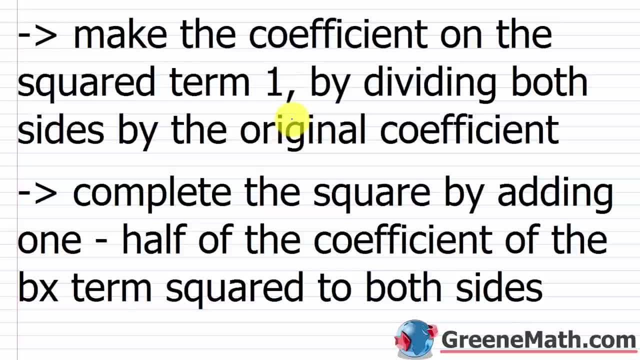 6x squared or 10x squared or 9x squared where you're going to have to deal with that. But you want the coefficient on the squared term to be one. All right, so here comes the next step. 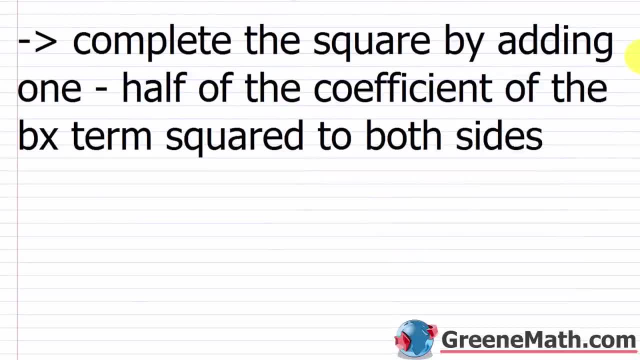 And this is the one that everybody gets wrong when they first start out. You're going to complete the square by adding one half of the coefficient of the bx term squared to both sides. Let me just reread that. 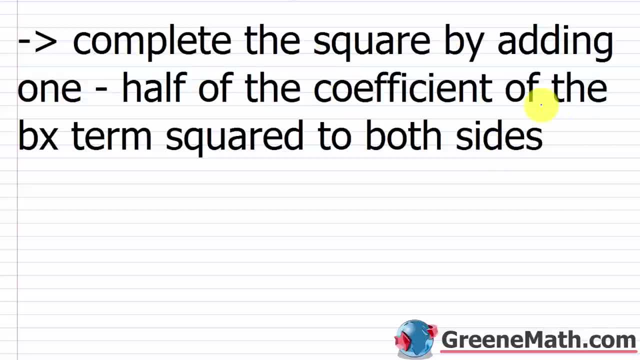 Complete the square by adding one half of the coefficient of the bx term squared to both sides. Complete the square by adding one half of the coefficient of the bx term squared to both sides. 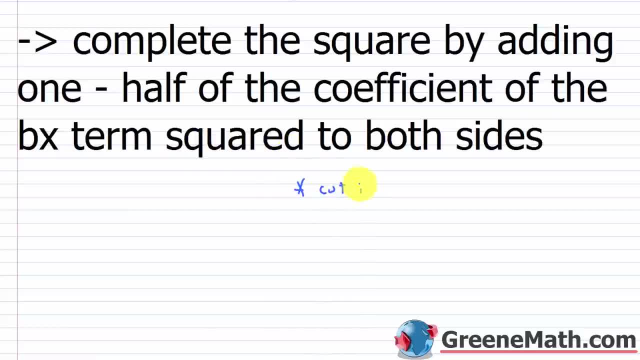 So I want you to write in your notes, cut it in half, then square it. This is how my eighth grade teacher taught it to me. 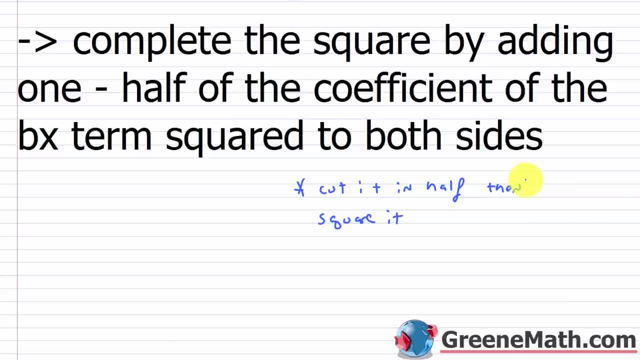 And it's stuck in my head for so, so many years. She would say, cut it in half and square it. 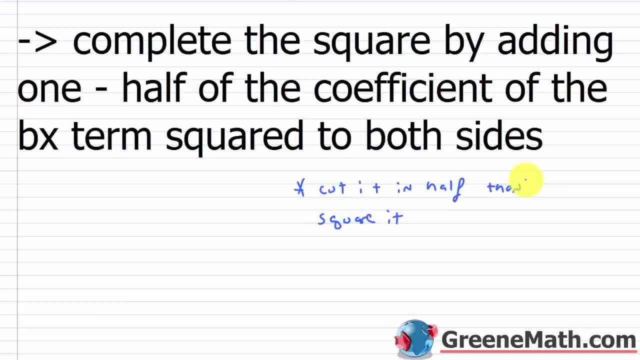 Okay, so every time that I would go to a problem and I struggled with this, I remember, what do I do? Cut it in half and square it. Cut it in half and square it. Just keep repeating that to yourself. And then completing the square will just be, you know, many years from now, 10 years from now, you're, you know, going to help your kid on their homework. And how do I complete the square? Cut it in half and square it, okay? Very, very good technique to remember this. 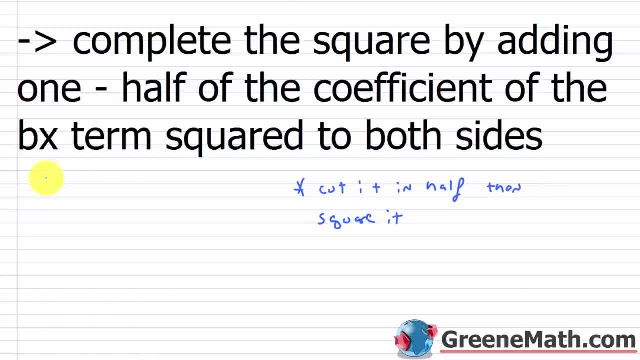 You may say, what is the bx term? This is just your term where the variable has an exponent of one. 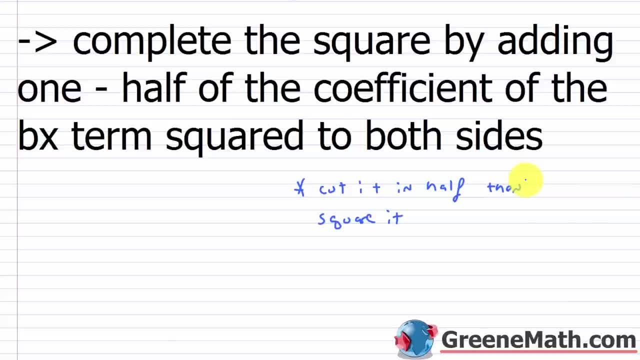 in my head for so, so many years. She would say: cut it in half and square it. Okay. so every time that I would go to a problem and I struggled with this, I remember what do I do? Cut it in half and square it. 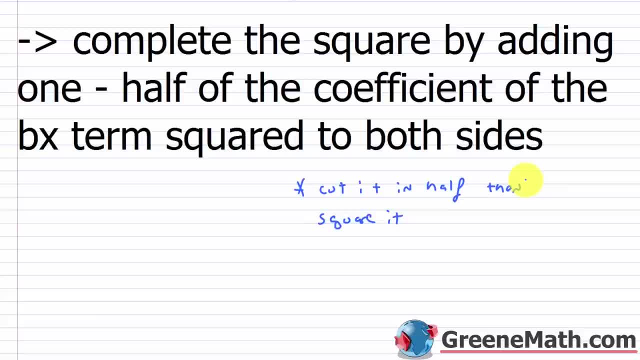 Cut it in half and square it. Just keep repeating that to yourself and then completing the square will just be. you know, many years from now, 10 years from now, you're, you know, going to help your kid on their homework. And how do I complete the square? Cut it in half and 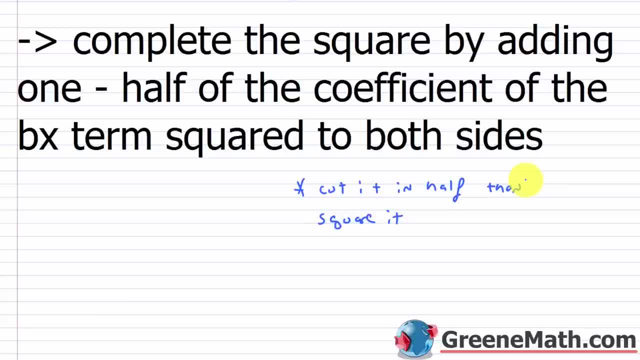 square it. Okay, very, very good technique to remember this. You may say: what is the bx term? This is just your term, where the variable has an exponent of one. Sometimes in your book, if you're reading the procedure there, it'll say the first degree. Okay, it just. 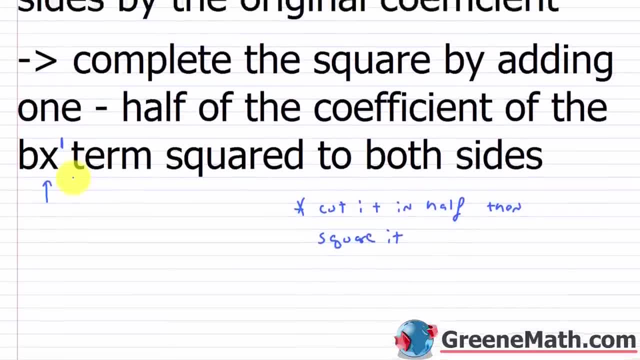 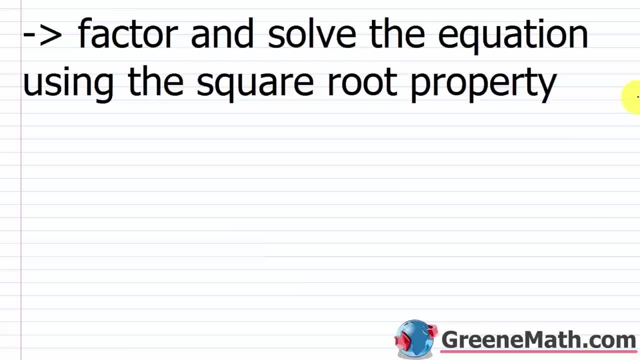 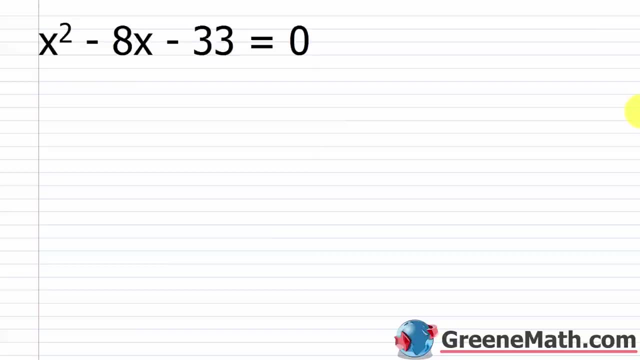 means that the exponent on the variable is a one. Then, once you've gotten through these previous steps, the final thing you're going to do is you're going to factor and solve the equation using the square root property. All right, so let's start out with our first example, And I gave you one that was really. 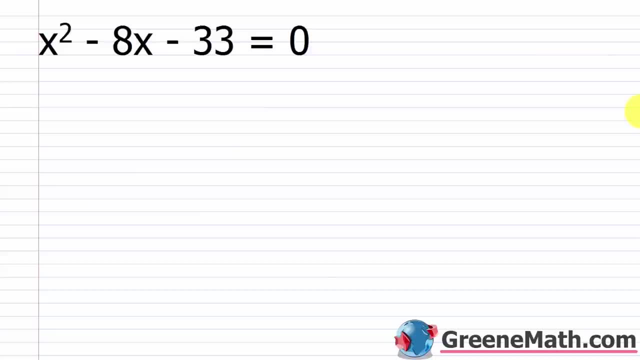 really easy. In fact, I gave you one that was really really easy. In fact, I gave you one that you could solve using factor. So if you wanted to pause the video and factor this, in fact we can just do it really quickly. We can have an x here and an x here: give. 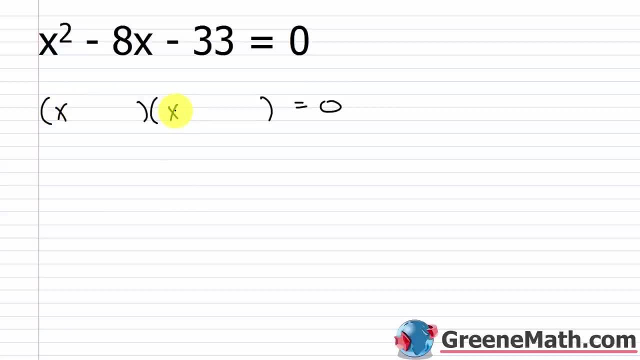 me two integers whose sum is negative eight and whose product is negative 33.. Well, I know I could do negative 11 and positive 30. So negative 11 and positive three. we know at this point that the solutions would be: x is equal to 11.. And then we're going to. do negative 11 and positive 30. So negative 11 and positive 30. We know at this point that the solutions would be: x is equal to 11.. And then we're going to do negative 11 and positive 30. We know at this point that the solutions would be: x is equal to 11.. And 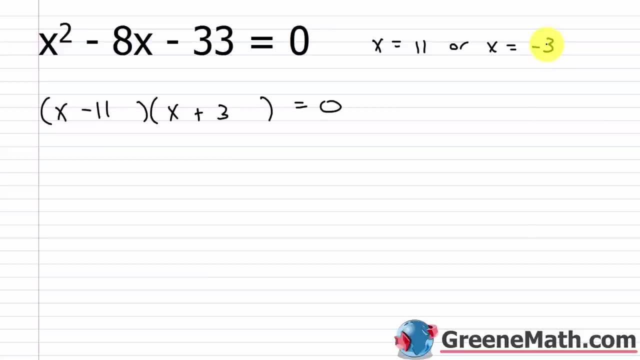 then we're going to do negative 11 and positive 30.. So negative 30. So the solution would be: x is equal to 11, or x is equal to negative three. All right, we can eyeball that and see it at this point, hopefully. So let's not use this, though. let's use our completing. 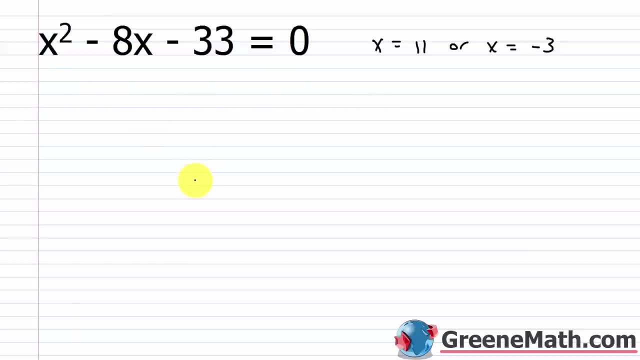 the square method And let's start out at step number one. So for step number one, we want to write the quadratic equation where the variable terms x, squared and BX are on one side and the constant is on the other. So in other words, 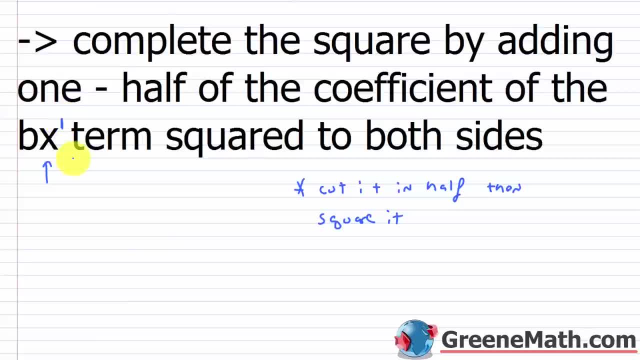 Sometimes in your book, if you're reading the procedure there, it'll say the first degree, okay? It just means that the exponent on the variable is a one. 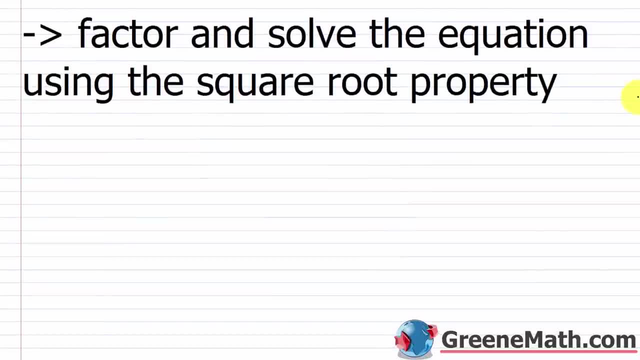 Then once you've gotten through these previous steps, the final thing you're going to do is you're going to factor and solve the equation using the square root property. 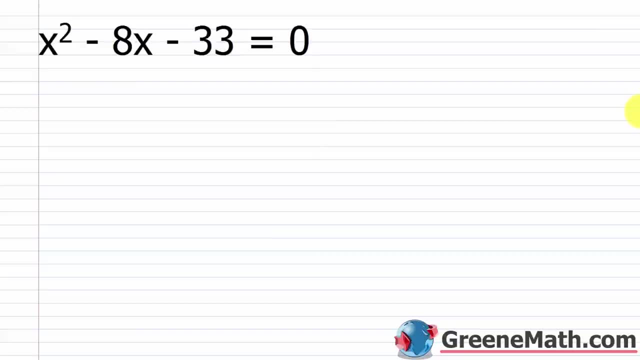 All right, so let's start out with our first example. And I gave you one that was really, really easy. In fact, I gave you one that you could solve using factor. So if you wanted to pause the video and factor this, in fact, we can just do it really quickly. We can have an x here and an x here. 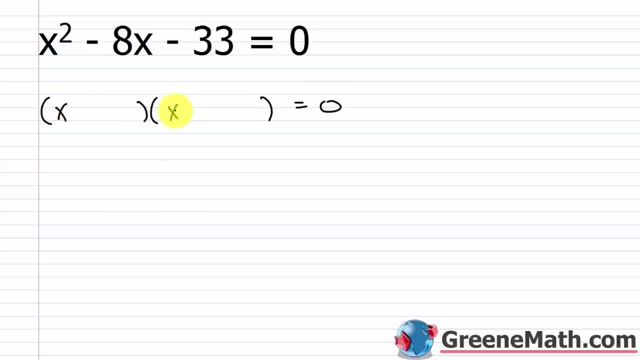 Give me two integers whose sum is negative eight and whose product is negative 33. Well, I know I could do negative 11 and positive 30. 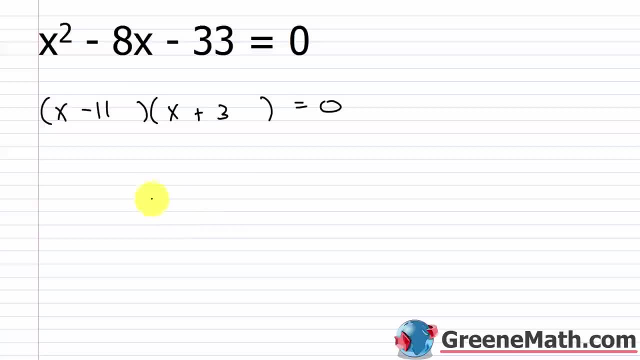 So negative 11 and positive three. 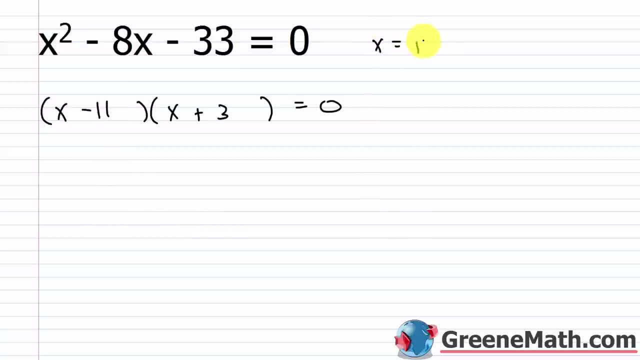 We know at this point that the solutions would be x is equal to 11 or x is equal to negative three. All right, we can eyeball that and see it at this point, hopefully. 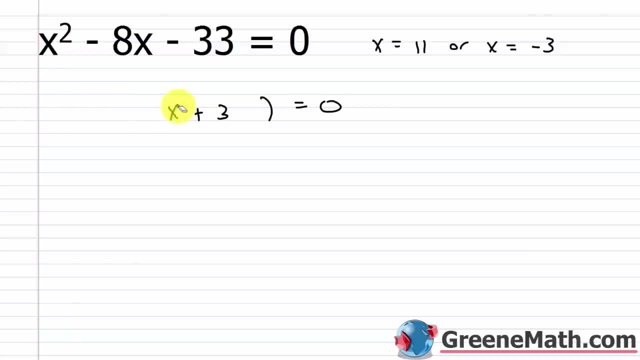 So let's not use this, though. Let's use our completing the square method. 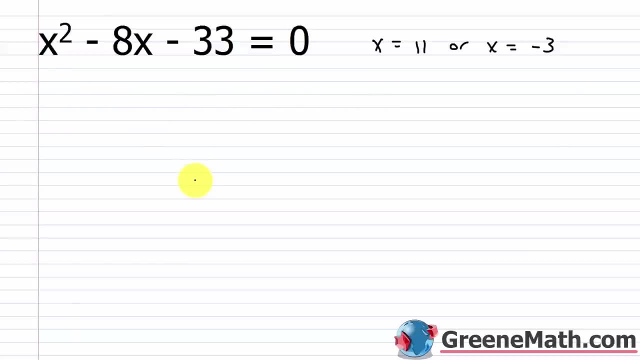 And let's start out at step number one. So for step number one, we want to write the quadratic equation where the variable terms ax squared and bx are on one side, and the constant is on the other. So in other words, these are your variable terms. 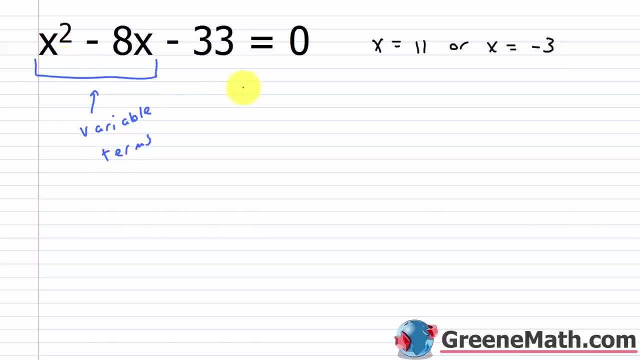 I want them by themselves. So what I've got to do is some basic algebra, and I'm going to add 33 to both sides of the equation. So that's going to give me x squared minus eight x is equal to 33. 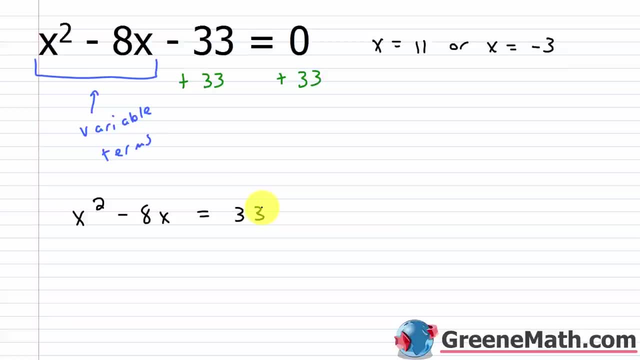 Now, the next thing is to make the coefficient on the square term one. But on the square term here, I already have a coefficient of a one. So I can just skip that. 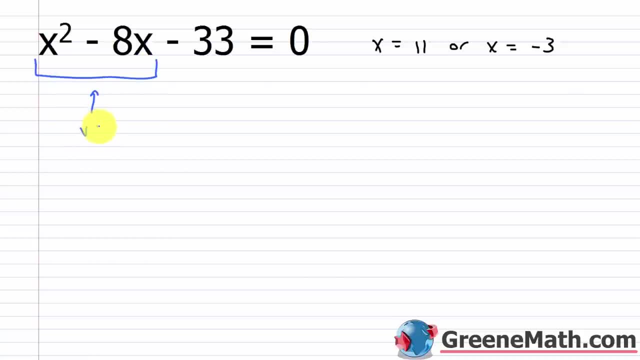 These are your variable terms. I want them by themselves. So what I've got to do is some basic algebra and I'm going to add 33 to both sides of the equation. So that's going to give me x squared minus 8x is equal to 33.. 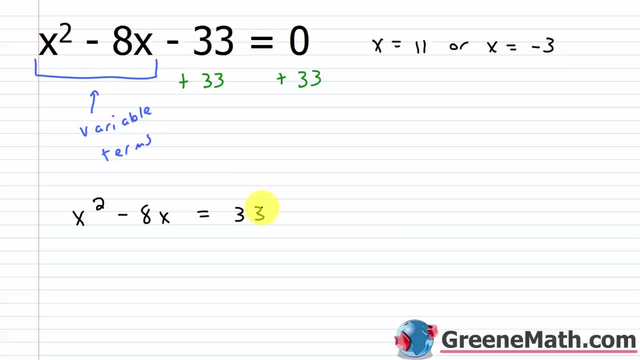 Now the next thing is to make the coefficient on the squared term 1, but on the squared term here I already have a coefficient of a 1, so I can just skip that, And in the case of algebra 1,, most of your problems will be pretty easy. 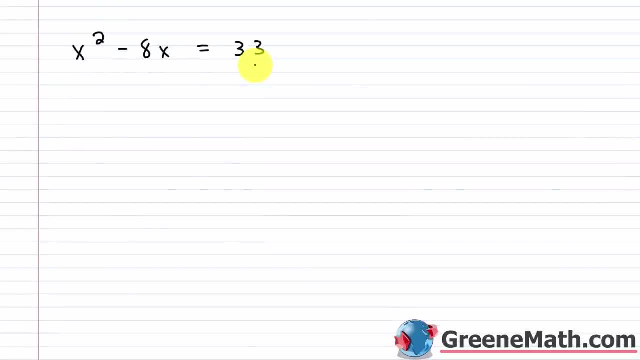 where you don't have to deal with that. Pretty much towards the end of your section on this you'll get a few of them, but mostly this is going to occur in algebra 2.. Now the next thing I want to do is complete the square. 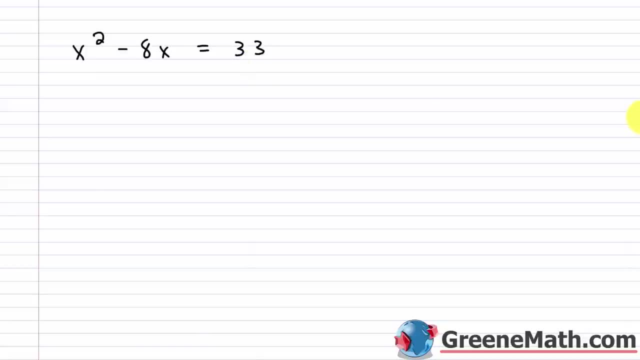 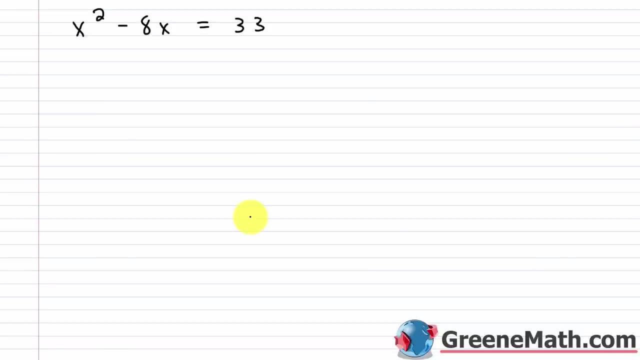 When I complete the square, it's the most kind of tedious thing that you're going to do because you have a lot of things to do. You have a lot of things that are going on, So let's kind of go slowly here. So we complete the square by adding 1 half of the coefficient of the bx term squared to both sides. 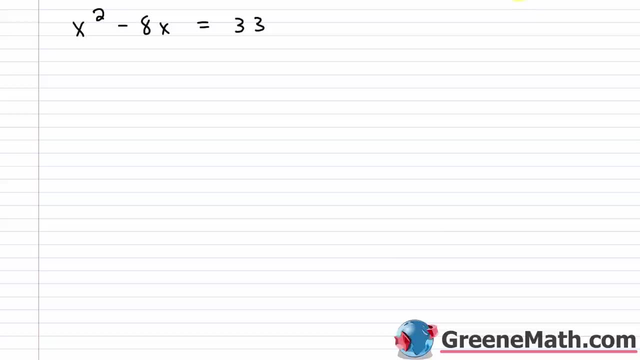 This is where you hear me say: cut it in half and square it. So this is your coefficient for the bx term. Basically you're x raised to the first power. So if I cut it in half, meaning I multiply negative 8 by 1 half. 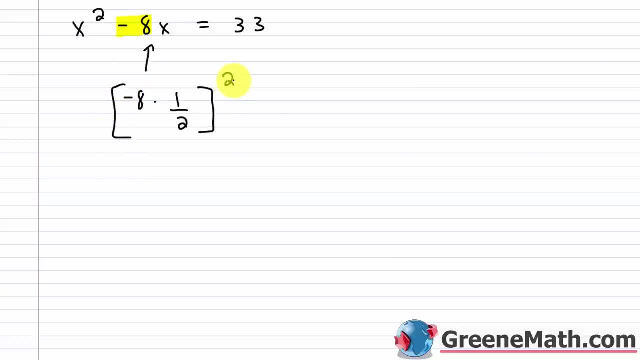 and I square that, I'm going to get what This is going to be. equal to negative 8 times 1. half is negative 4.. So I'd have negative 4 squared, So this is equal to 16.. So, essentially, I want to add 16 to each side of the equation. 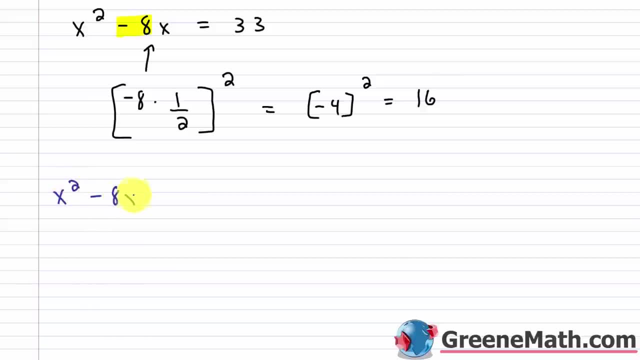 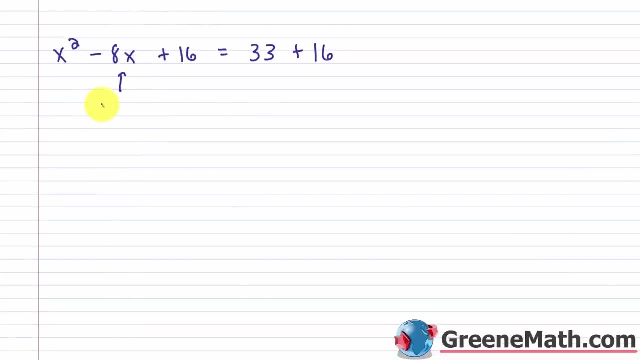 So I'd have: x squared minus 8x plus 16 is equal to 33 plus 16.. Now what I've done here is I've just completed the square. If you'll notice, now, this is a perfect square. This is a perfect square trinomial. 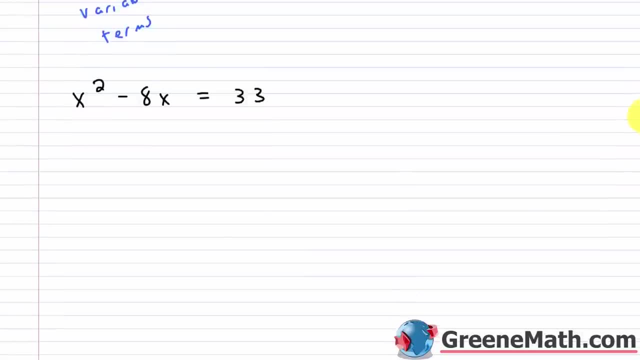 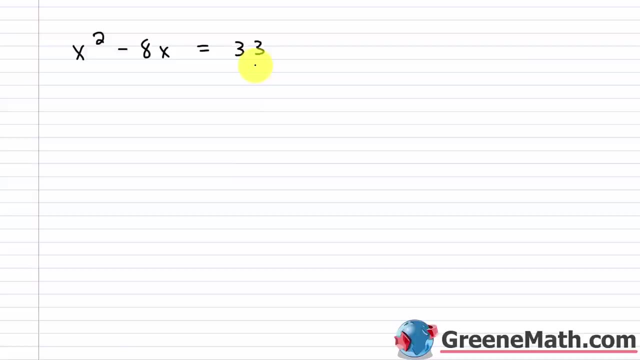 And in the case of algebra one, most of your problems will be pretty easy where you don't have to deal with that. Pretty much towards the end of your section on this, you'll get a few of them. But mostly this is going to occur in algebra two. Now, the next thing I want to do is complete the square. 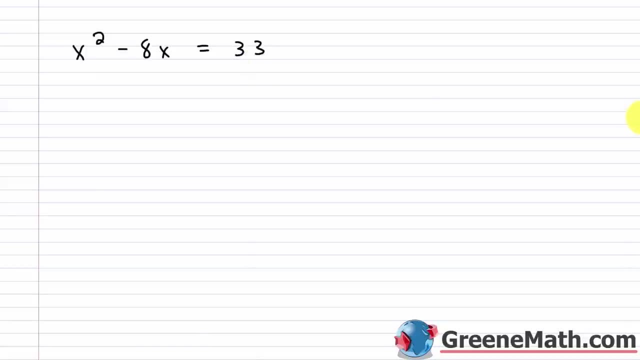 When I complete the square, it's the most kind of tedious thing that you're going to do because you have a lot of things that are going on. So let's kind of go slowly here. 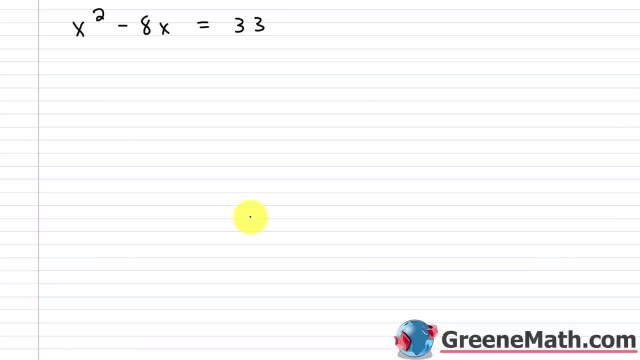 So we complete the square by adding one half of the coefficient of the bx term. 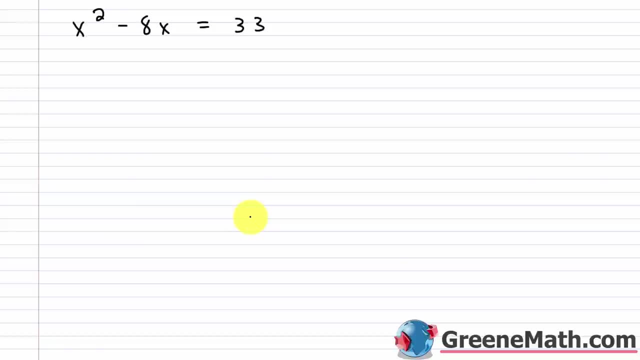 So I'm going to take the bx term and I'm going to take the bx term squared to both sides. Okay. 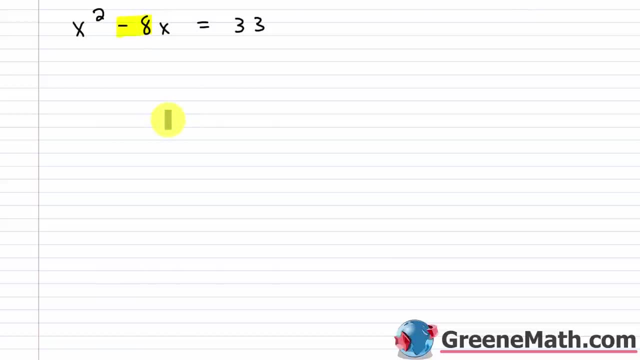 This is where you hear me say, cut it in half and square it. So this is your coefficient for the bx term. Okay. 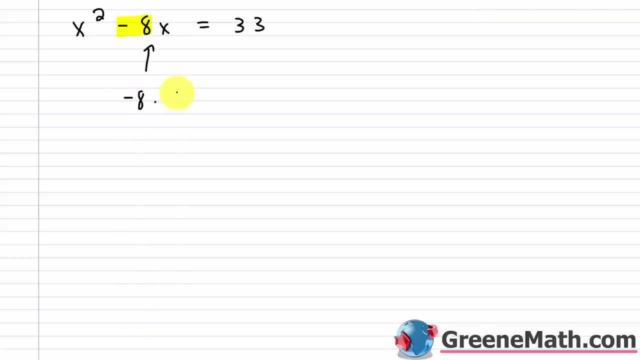 You're basically your x raised to the first power. So if I cut it in half, meaning I multiply negative eight by one half and I square that, 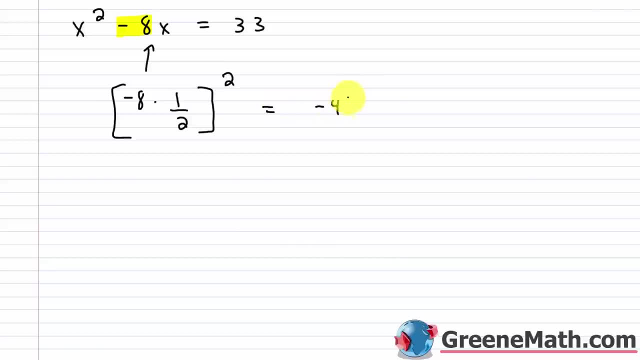 I'm going to get what this is going to be equal to. So it's going to be eight squared. So this is equal to 16. 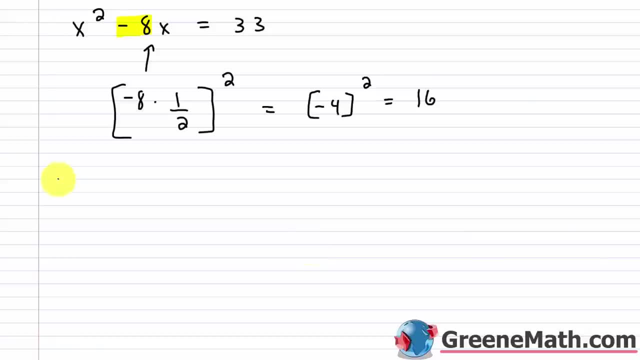 So essentially I want to add 16 to each side of the equation. So I'd have x squared minus eight x plus 16 is equal to 33 plus 16. Now, what I've done here is I've just completed the square. 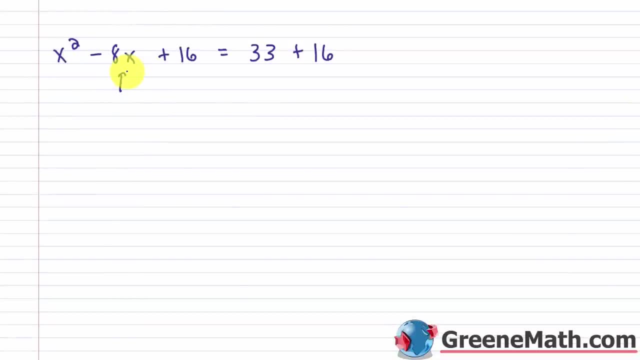 If you'll notice now, this is a perfect square. 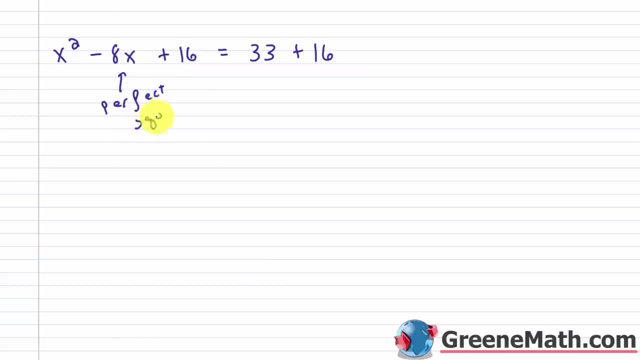 This is a perfect square. Okay. 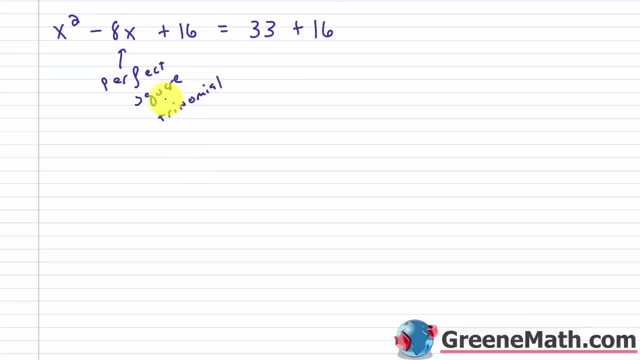 trinomial. So I know that this is going to factor into a binomial squared, and it would be what? It would be x minus, I have that minus there, and the square root of 16 would be 4. So x minus 4, that quantity squared, is equal to over here 33 plus 16 is 49. So now I have something where I can use my square root property, and in the final step it says to factor, which we just did, and then to solve using our square root property. So I'm going to take the square root of this side, and then over here I'm going to put plus or minus the square root of this side. And so what I'm going to have is x minus 4, because this would cancel with this, is equal to plus or minus the square root of 49 is 7. So this gives me two different scenarios. 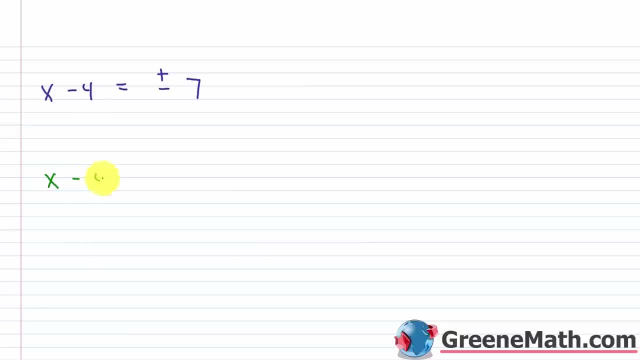 Two different scenarios. It gives me x minus 4 is equal to 7, or x minus 4 4 is equal to negative 7. 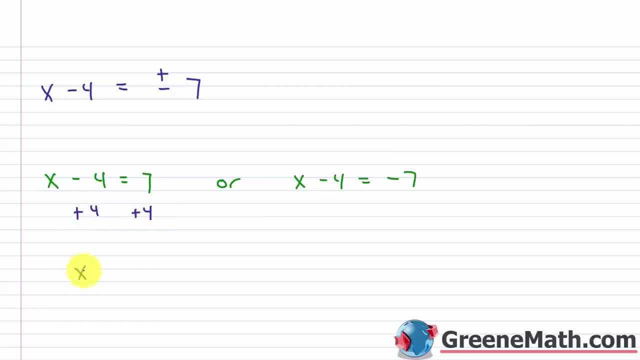 So then I solve this, add 4 to each side of the equation, I get x equals 11, or add 4 to each side of the equation, I get x is equal to negative 3. 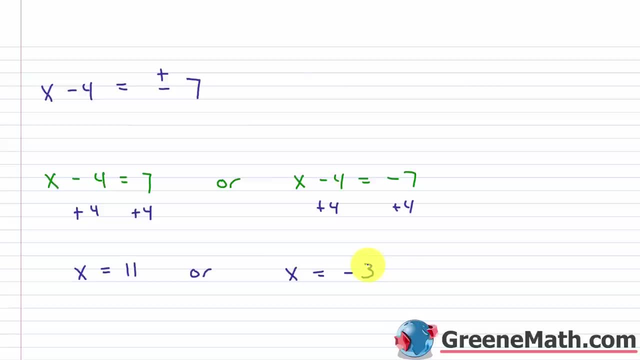 Now you'll recall at the very beginning of this problem I solved it using factoring and I got the same thing. And you might say, why in the world would you use completing the square, that took way longer than factoring. Well in a lot of cases you're not going to be able to use factoring, and additionally we're not going to be using completing the square for more than a week in our Algebra 1 class. 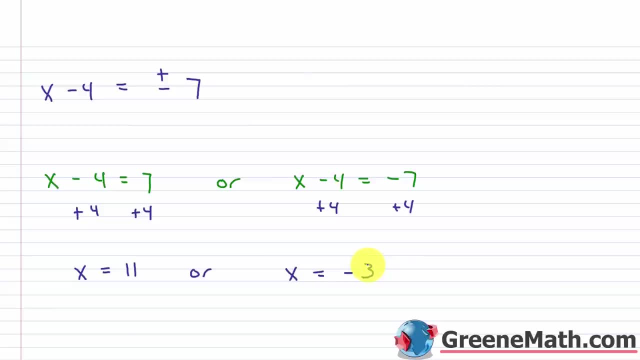 In the next lesson we're going to learn about something that was a quadratic formula, and once you learn that you're not going to use factoring, and you're not going to use completing the square, you're pretty much going to use that. 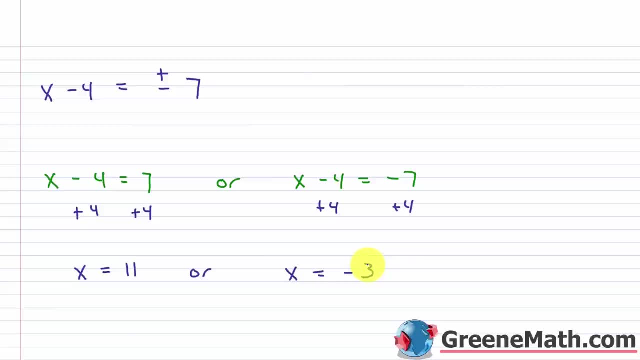 You just plug numbers into a generic formula and it spits out an answer for you. But before you can get to that you need to understand this here. 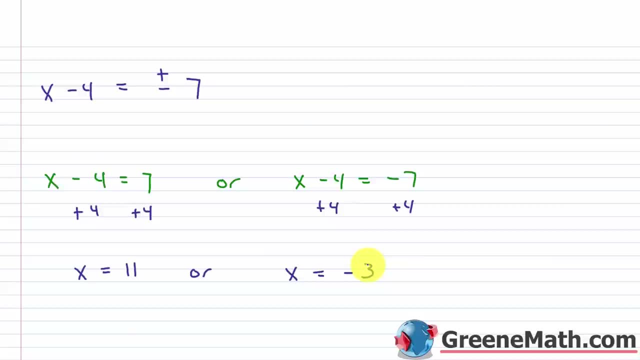 So in the interest of time I'm not going to check this, normally I check everything, but we have a lot more time. We have a lot more problems that we want to cover, I don't want to make the video too long. 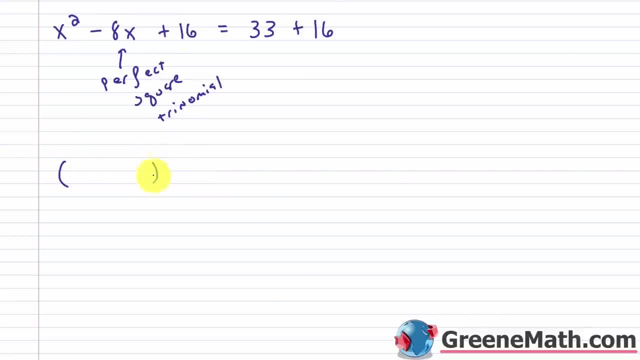 So I know that this is going to factor into a binomial squared And it would be what It would be: x minus- I have that minus there- And the square root of 16 would be 4.. So x minus 4 of that quantity squared is equal to over here. 33 plus 16 is 49.. 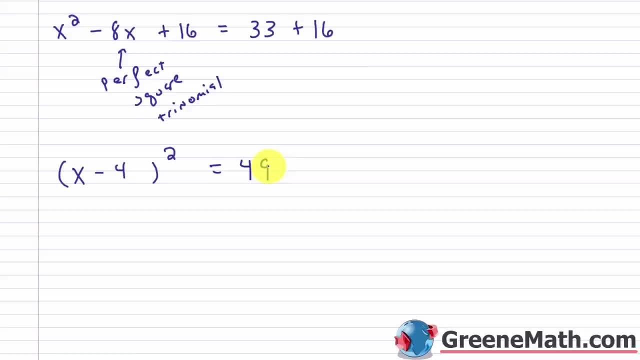 So now I have something Where I can use my square root property And in the final step it says to factor, which we just did, And then to solve using our square root property. So I'm going to take the square root of this side. 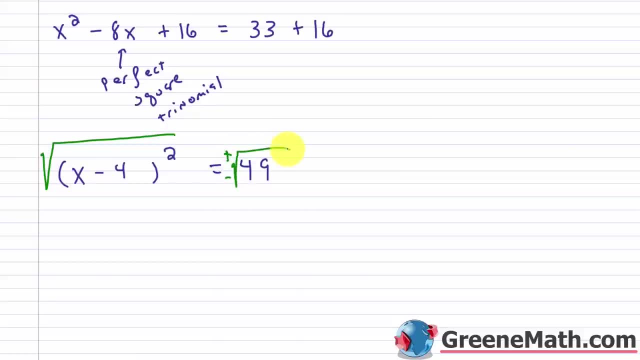 And then over here I'm going to put plus or minus the square root of this side, And so what I'm going to have is x minus 4, because this would cancel with. this is equal to plus or minus. the square root of 49 is 7.. 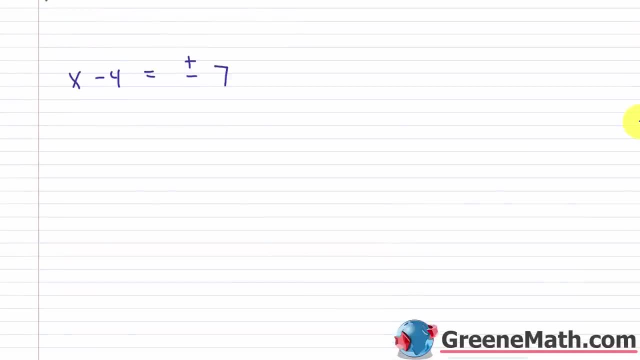 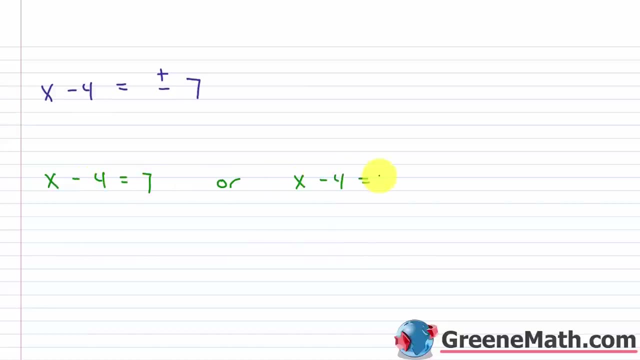 So this gives me two different scenarios. It gives me x minus 4 is equal to 7, or x minus 4 is equal to negative 7.. So then I solve this. add 4 to each side of the equation, I get x equals 11.. 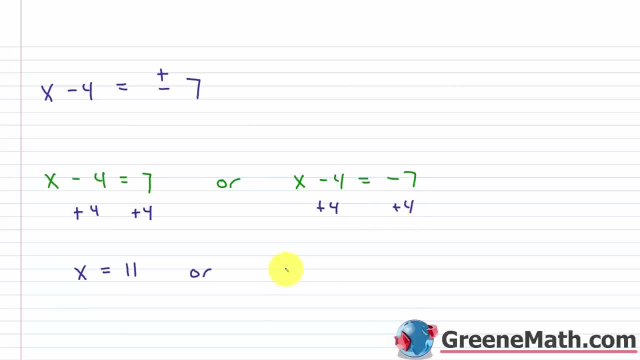 Or add 4 to each side of the equation I get x is equal to negative 3.. Now you'll recall, at the very beginning of this problem, I solved it using factoring and I got the same thing. And you might say, why in the world would you use completing the square root? 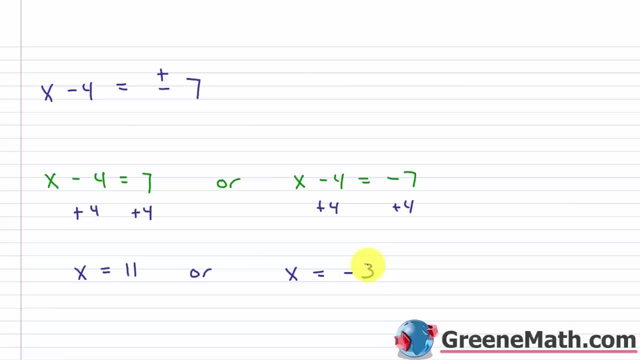 It took way longer than factoring. Well, in a lot of cases you're not going to be able to use factoring And, additionally, we're not going to be using completing the square for more than a week in our Algebra 1 class. 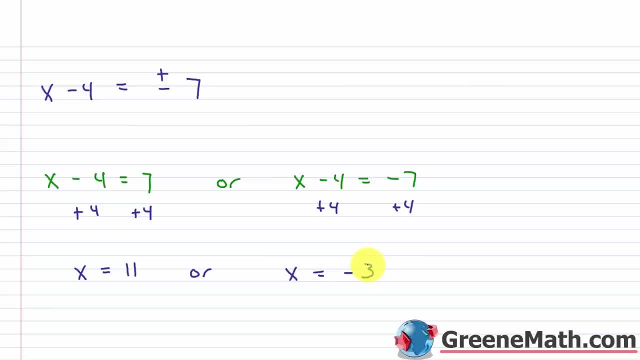 In the next lesson we're going to learn about something that was a quadratic formula, And once you learn that you're not going to use factoring and you're not going to use completing the square, Pretty much- you're going to use that. 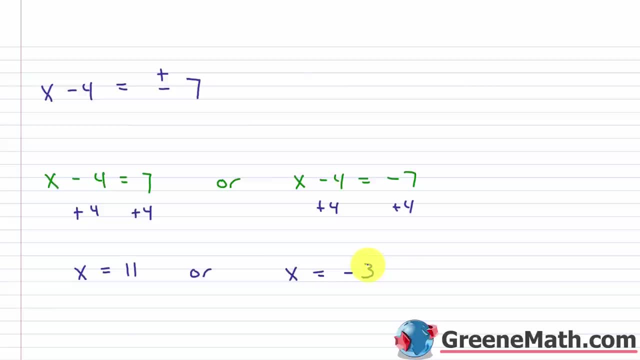 You just plug numbers into a generic formula and it spits out an answer for you, But before you can get to that, you need to understand this. So, in the interest of time, I'm not going to check this. Normally I check everything, but we have a lot more problems that we want to cover. 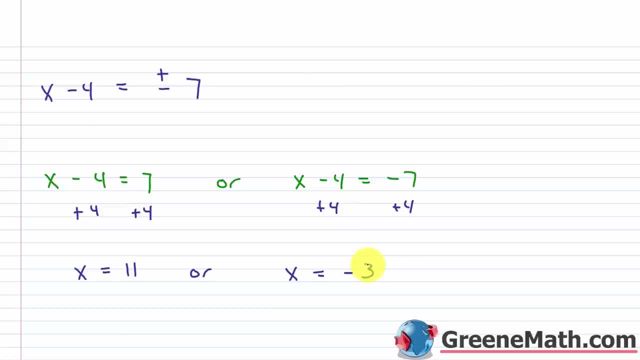 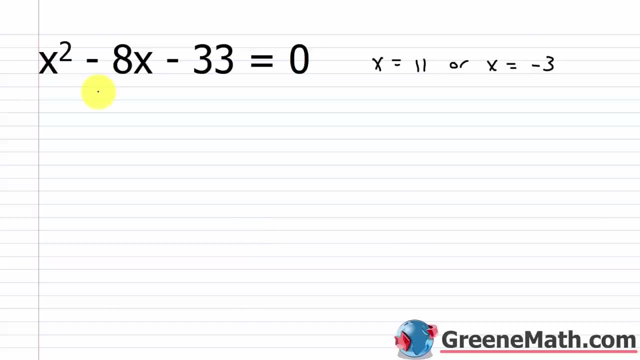 I don't want to make the video too long, So pause the video, go back up to the original equation and plug in an 11 for x and plug in a negative 3 for x, And you'll see that both of these would be a valid solution. 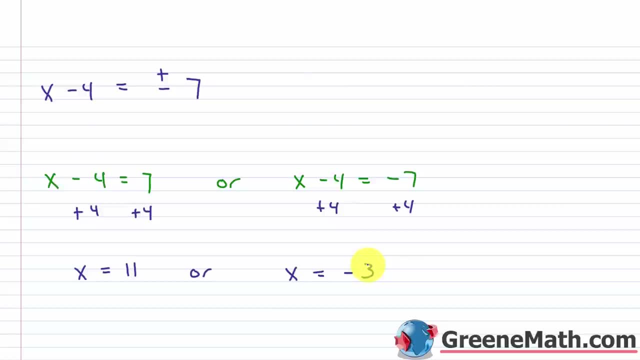 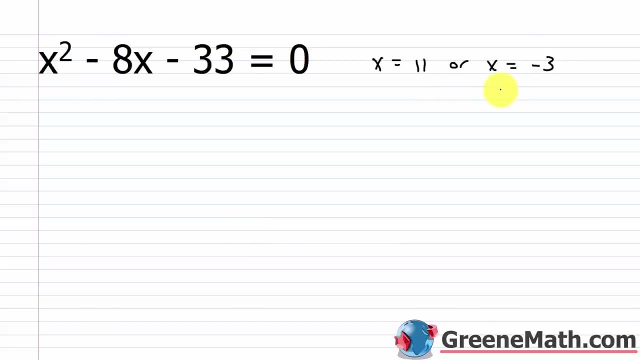 So pause the video, go back up to the original equation, and plug in an 11 for x, and plug in a negative 3 for x, and you'll see that both of these would be a valid solution. Alright let's take a look at the next one. 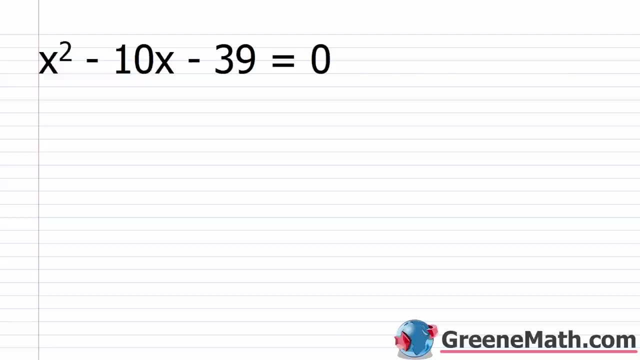 So we have x squared minus 10x minus 39 equals 0. So again the first thing I do is I move the variable terms on one side, and I move the constant to the other. So in this case I would add 39 to each side of the equation, and I would have x squared minus 10x is equal to 39. And then the next thing is to make sure the coefficient on the square term is 1, in this case we already have that. 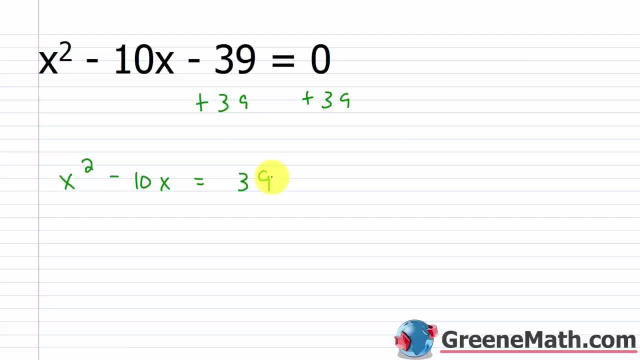 Then we're going to complete the square by adding one half of the coefficient of the bx term squared to both sides. 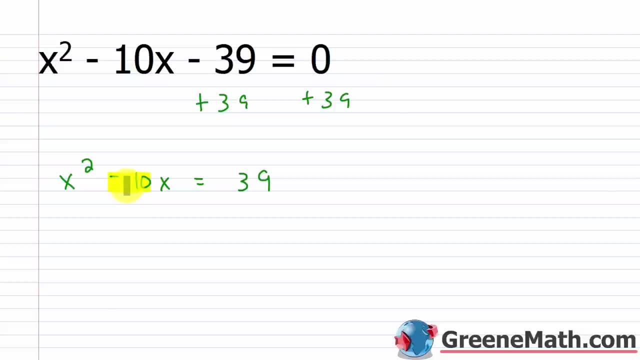 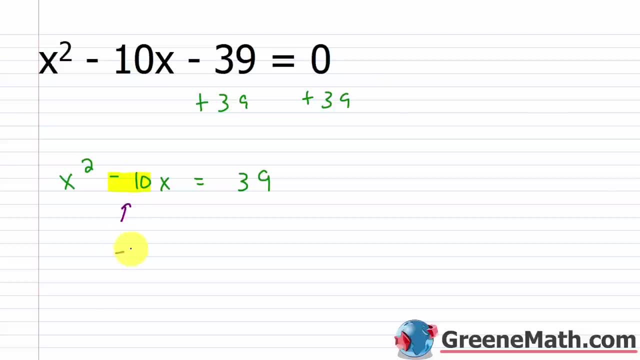 Cut it in half and square it. So negative 10, cut it in half, that's like multiplying by half, and then square it. So this is equal to, that would be negative 10 over 2 is negative 5, negative 5 squared is 25. 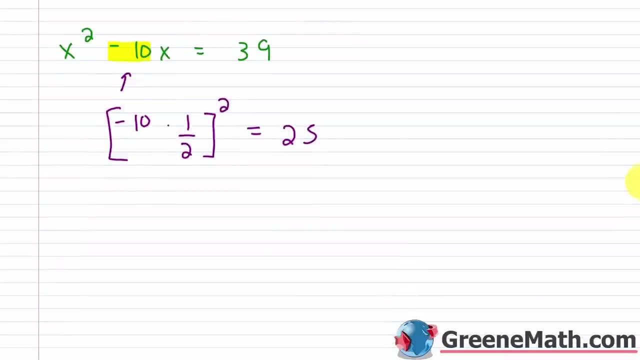 So I'm going to add 25 to each side of the equation. So I'm going to have x squared minus 10x plus 25 is equal to 39. 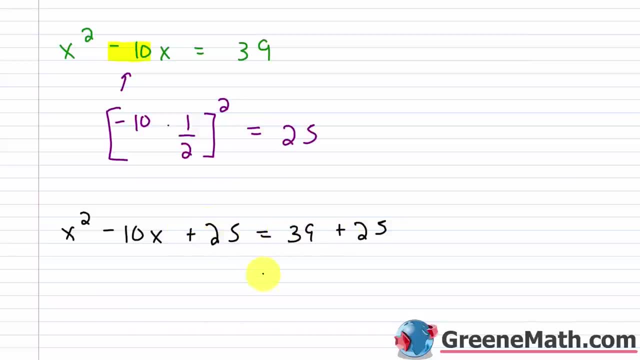 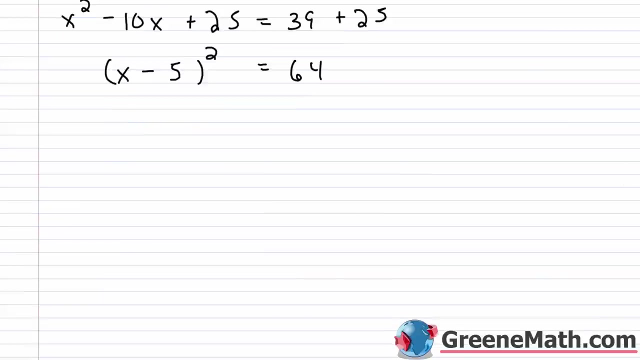 to 39 plus 25. And 39 plus 25 is 64. And over here, I would factor this. This is now a perfect square trinomial. So it can be factored into a binomial squared. And this would be x. I have minus there. Square root of 25 is 5. So x minus 5, that quantity squared. So now we can use our square root property. And let me just rewrite this. We have x minus 5. This quantity squared is equal to 64. And I want to take the square root of this side. And then I want to do plus or minus the square root of this side. And so what I'm going to get is this cancels with this of x minus 5 is equal to plus or minus the square root of 64 is 8. So I would have two different scenarios. 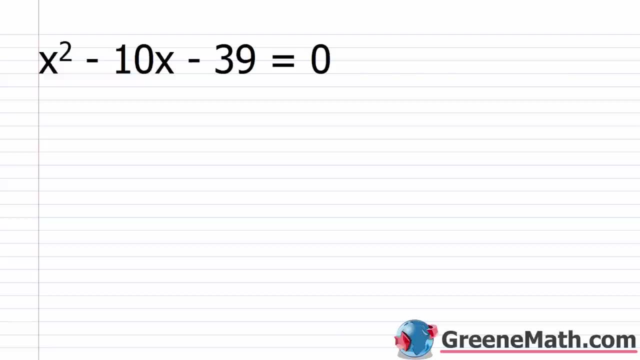 Alright, let's take a look at the next one. So we have x squared minus 10x minus 39 equals 0.. So, again, the first thing I do is I move the variable terms on one side and I move the constant to the other. 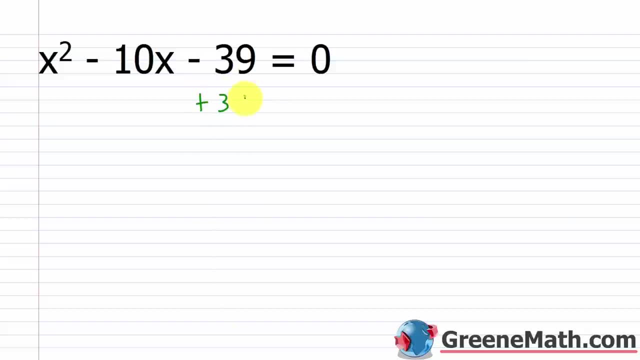 So in this case I would add 39 to each side of the equation And I would have x squared minus 10x is equal to 39.. And then the next thing is to make sure the coefficient on the square term is 1.. 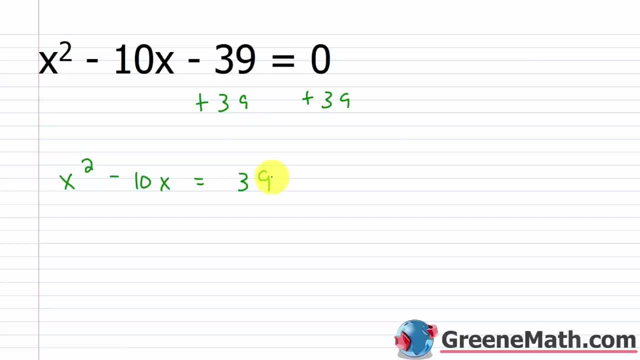 In this case we already have that. Then we're going to complete the square by adding one half of the coefficient of the bx2.. And then we're going to add the bx term, squared to both sides. So, again, what I want to do: cut this in half and square it. 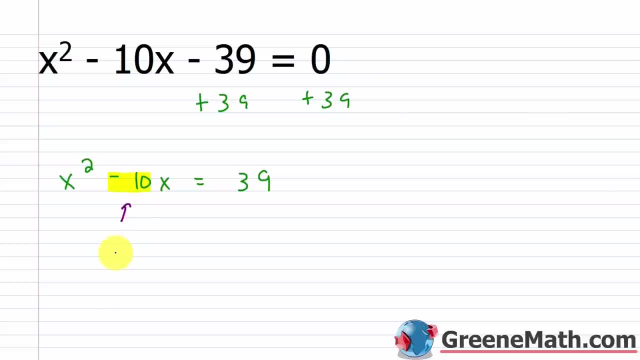 Cut it in half and square it. So negative 10, cut it in half, that's like multiplying by half and then square it. So this is equal to that would be negative. 10 over 2 is negative 5, negative 5 squared is 25.. 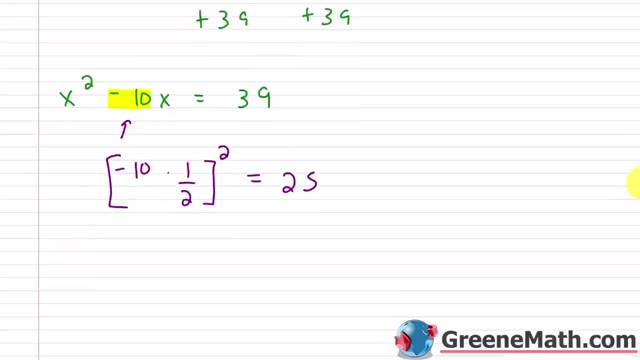 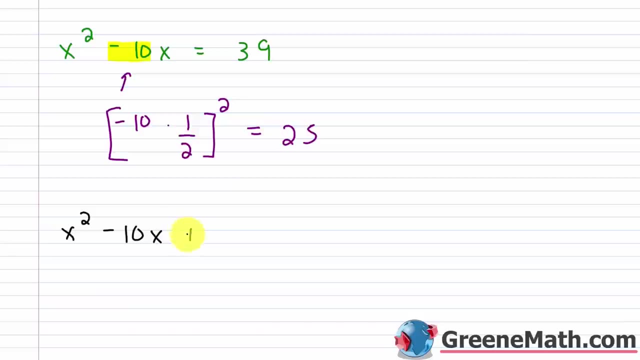 So I'm going to add 25 to each side of the equation. So I'm going to have x squared minus 10x plus 25 is equal to 39 plus 25.. And 39 plus 25 is 64.. And over here I would factor this: 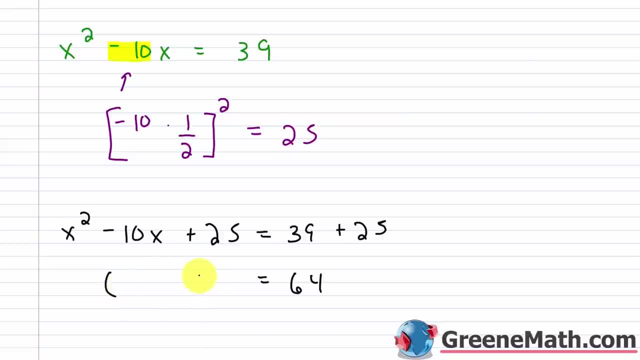 This is now a perfect square trinomial, So it can be factored into a binomial squared, And this would be x. I have minus there. squared, 25 is 5.. So x minus 5, that quantity squared. So now we can. 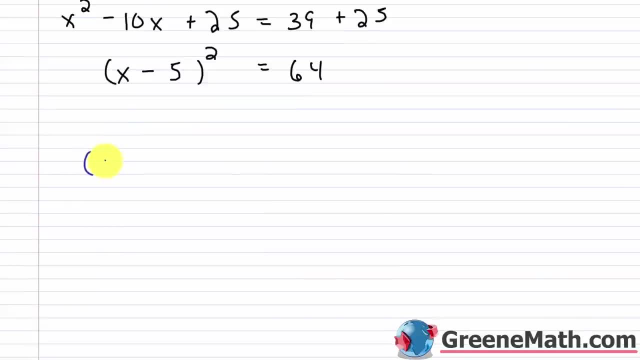 Now we can use our square root property and let me just rewrite this. We have x minus 5, this quantity squared is equal to 64. And I want to take the square root of this side and then I want to do plus or minus the square root of this side. 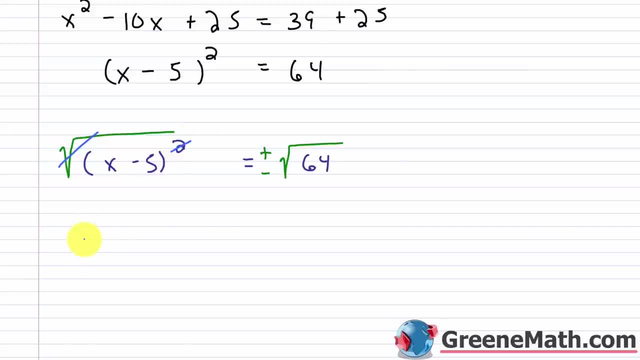 And so what I'm going to get is this: cancels with this of x minus 5 is equal to plus or minus. the square root of 64 is 8.. So I would have two different scenarios. x minus 5 is equal to 8.. 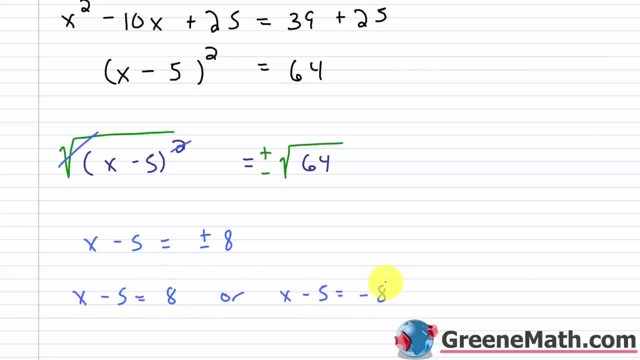 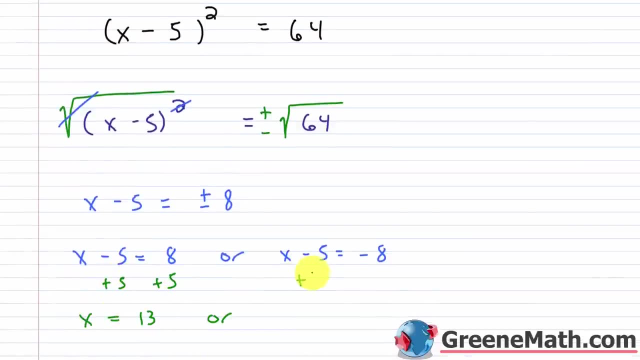 Or x minus 5 is equal to 8.. Or x minus 5 is equal to negative 8.. So we'd solve these. add 5 to each side of the equation here. Now we get x is equal to 13.. Add 5 to each side of the equation here. 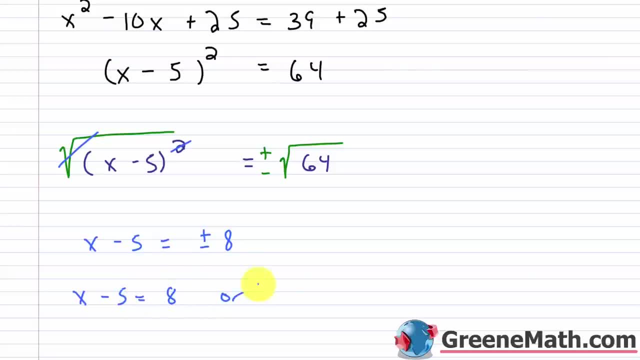 x minus 5 is equal to 8. Or x minus 5 is equal to negative 8. So we'd solve these, add 5 to each side of the equation here. 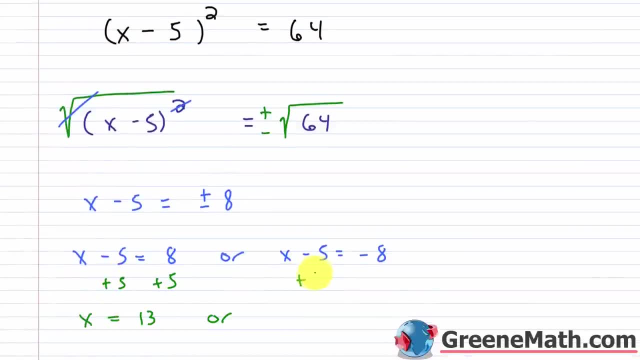 And I would get x is equal to 13. Add 5 to each side of the equation here. And I would get x is equal to negative 3. So again, in the interest of time, I'm not going to check these. So you can 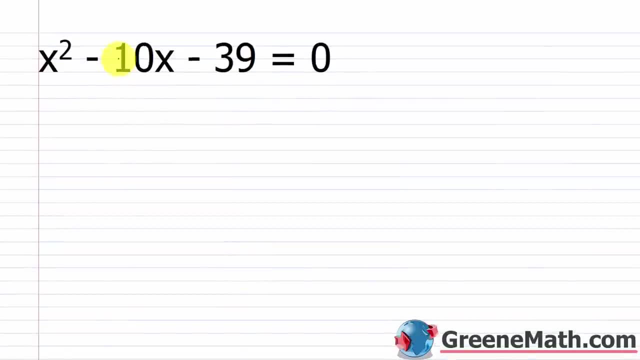 pause the video, come back to this original equation, x squared minus 10x minus 39 equals 0. 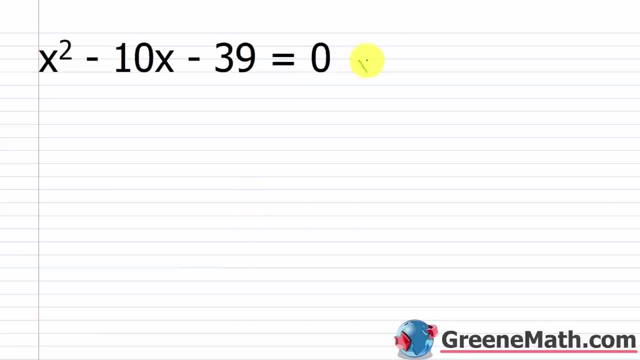 And then plug in for x. You had x equals 13. That's one solution. And then another solution, again, is x equals negative 3. In each case, you're going to see that the left and the right are going to be equal. And so those are two valid solutions. All right, let's take a look at another 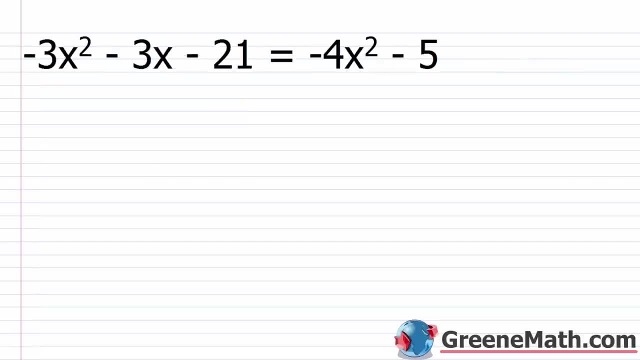 one. So we have negative 3x squared minus 3x minus 21 is equal to negative 4x squared minus 5. So knowing that I want all the variable terms on one side and all the constants on the other, if I add 4x squared to each side of the equation, this is going to go away. And on this side, I'm going to just have x squared. Then minus 3x. And what I want to do is I'm going to add 4x squared to each side of the equation. 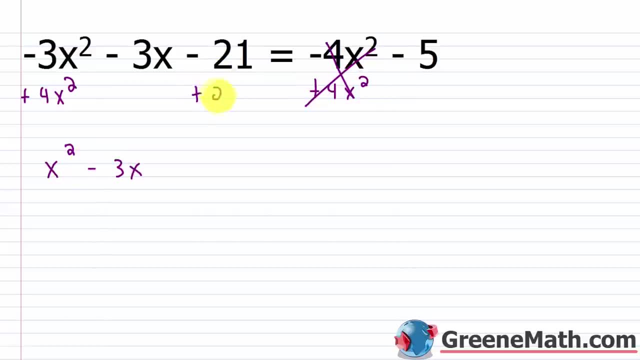 So what I want to do here, I'm going to move this over here. So let me add 21 to each side of the equation. That's gone. So this will be equal to negative 5 plus 21 is 16. So now I have x squared minus 3x equals 16. Now the coefficient on the x squared is a 1. So I don't need to do 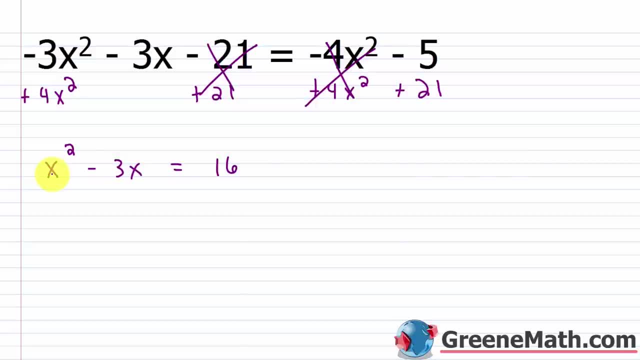 anything there. So now I want to move into my complete the square step. So I take the coefficient for the x squared. 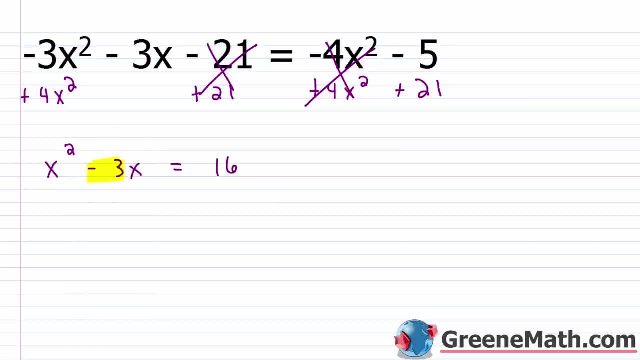 I take the first power here. So that's negative 3. I cut it in half and I square it. Cut it in half. So I multiply it by 1 half. And then I square it. 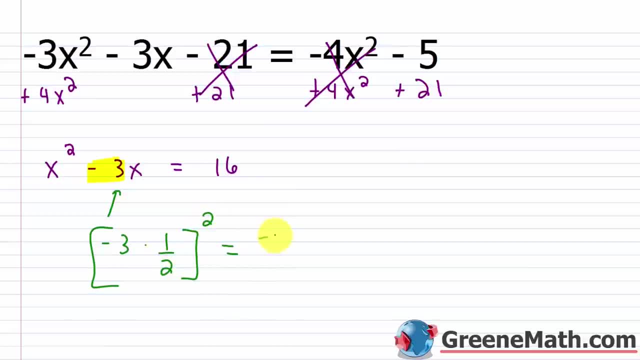 So negative 3 times 1 half is just negative 3 halves. 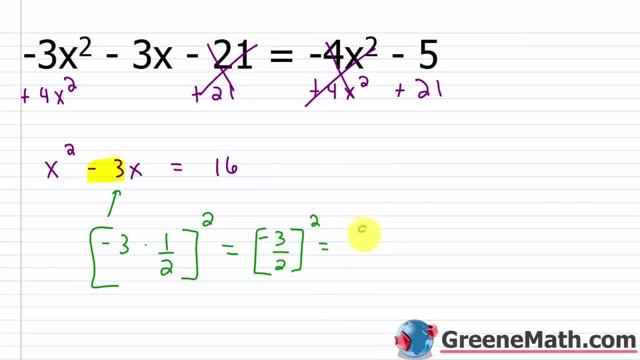 And then if I square that, I'm going to get 9 fourths. Okay, 9 fourths. So I'm going to be adding that to both sides of the equation. 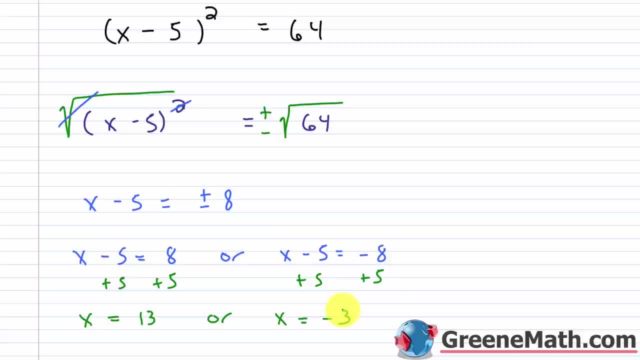 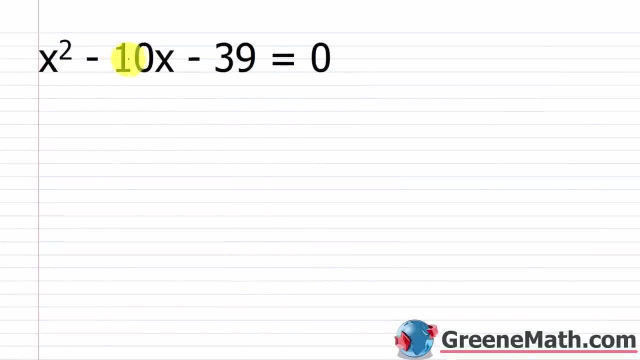 And now we get: x is equal to negative 3.. So again, in the interest of time, I'm not going to check these, So you can pause the video. come back to this original equation: x squared minus 10x minus 39 equals 0.. 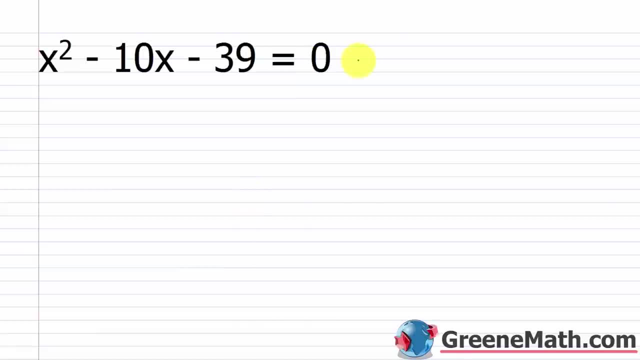 And then plug in for x, You had x equals 13. That's one solution, And then another solution again is x equals negative 3. In each case, you're going to see that the left and the right sides would be equal. 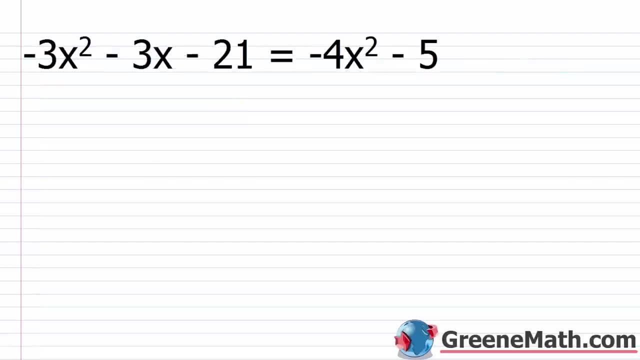 And so those are two valid solutions. All right, let's take a look at another one. So we have negative 3x squared minus 3x minus 21 is equal to negative 4x squared minus 5.. So, knowing that I want all the variable terms on one side and all the constants on the other, 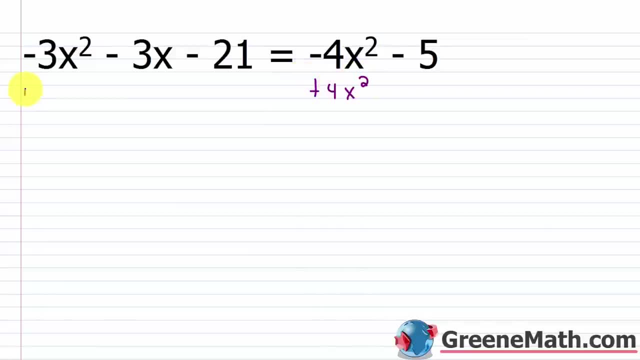 if I add 4x squared to each side of the equation, this is going to go away. Okay, I'm going to just have x squared, then minus 3x, And what I want to do here, I'm going to move this over here. 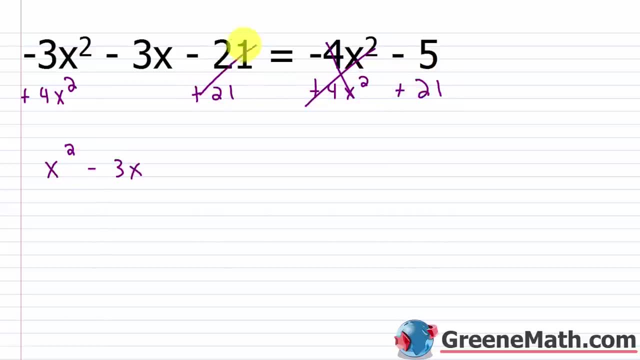 So let me add 21 to each side of the equation. That's gone. So this will be equal to negative. 5 plus 21 is 16.. So now I have: x squared minus 3x equals 16.. Now the coefficient on the x squared is a 1.. 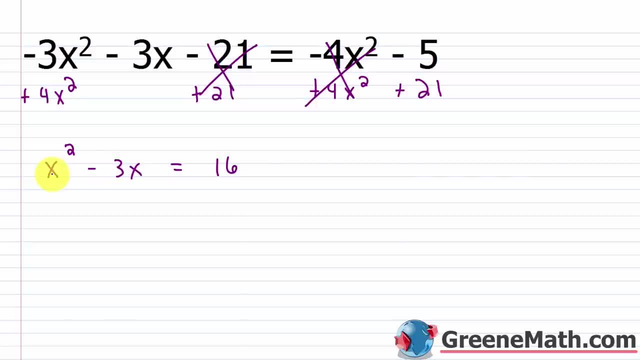 So I don't need to do anything there. So now I want to move into my complete equation. So now I want to move into my complete equation. So now I want to move into my complete the square step. So I take the coefficient for the x to the first power here. 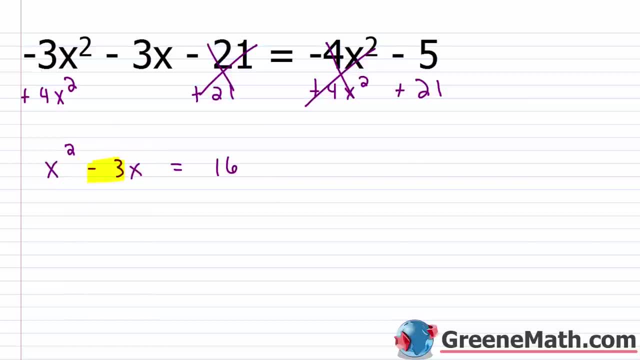 So that's negative 3. I cut it in half and I square it. Cut it in half, So I multiply it by 1 half And then I square it. So negative 3 times 1 half is just negative 3 halves. 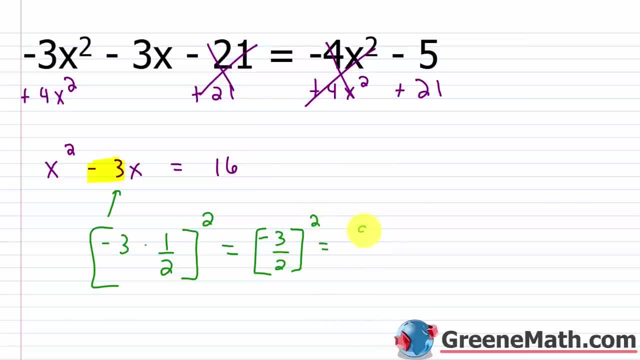 And then, if I square that, I'm going to get 9 fourths. Okay, 9 fourths, So I'm going to be adding that to both sides of the equation. So I'm going to add 9 fourths here. 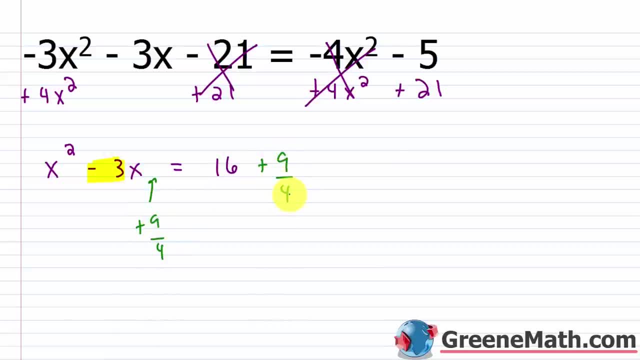 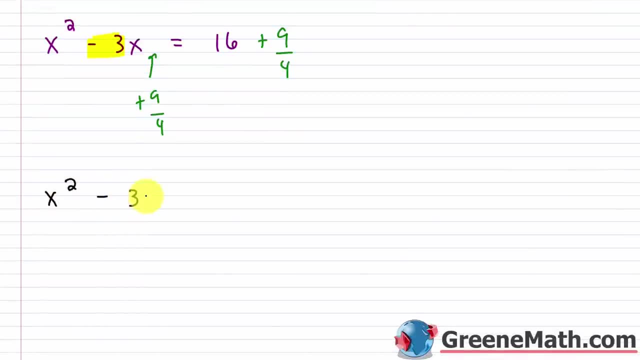 And I'm going to add 9 fourths here. Let me scroll down. So if I add that over here, I'll have x squared minus 3x plus 9 fourths. Then over here, if I get a common denominator going, I'll multiply this by 4 over 4.. 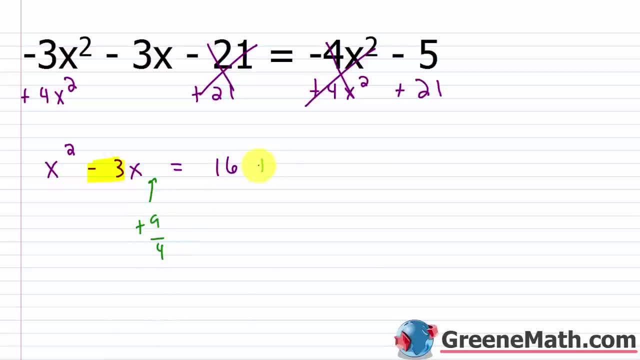 So I'm going to add 9 fourths here. And I'm going to add 9 fourths here. Let me scroll down. 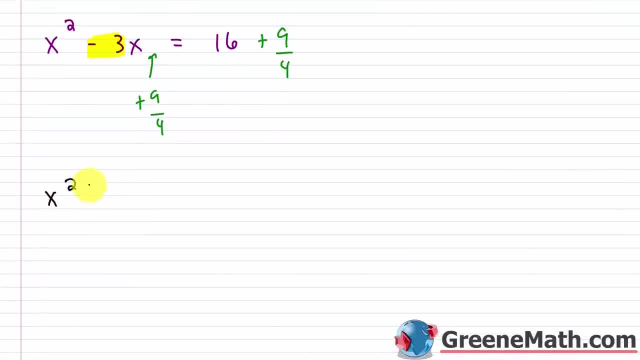 So if I add that over here, I'll have x squared minus 3x plus 9 fourths. Then over here, if I get a common denominator going, I'll multiply this by 4 over 4. 4 times 16 is of course 64. So I'd have 64 plus 9 over 4. And 64 plus 9 is 64. 73. So this would be 73 fourths. Now at this point, this is a perfect square trinomial. 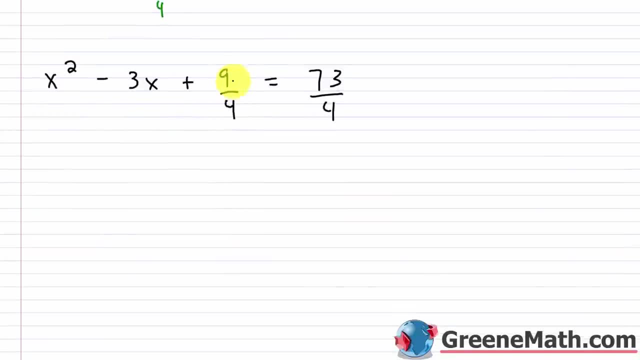 I can factor this. And I know a lot of you aren't used to seeing fractions when you go to factor stuff. It's not any more difficult. Just follow your pattern. So this is going to be x. You have a minus here. So this is minus. What's going to go in that position? Well, just take the square root of this. The square root of 9 is 3. And the square root of 4 is 2. So this is going to be 3 halves. And go ahead and boil that out if you don't believe me. You're going to end up with x squared minus 3x plus 9 fourths. OK. So this equals 73 fourths. And now we use our square root property. So I take the square root of this side and then plus or minus the square root of this side. And what I'm going to end up with is x minus 3 halves. arm. 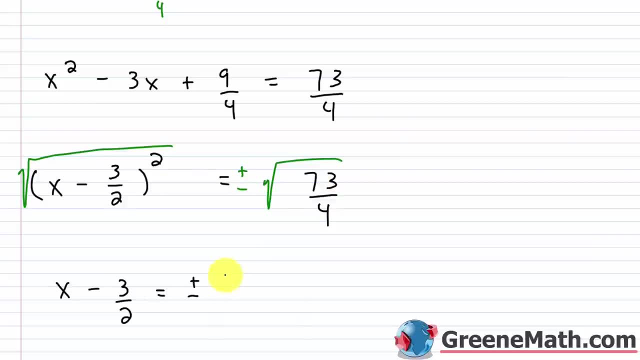 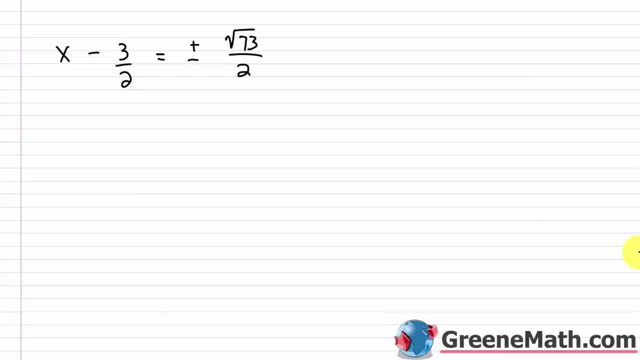 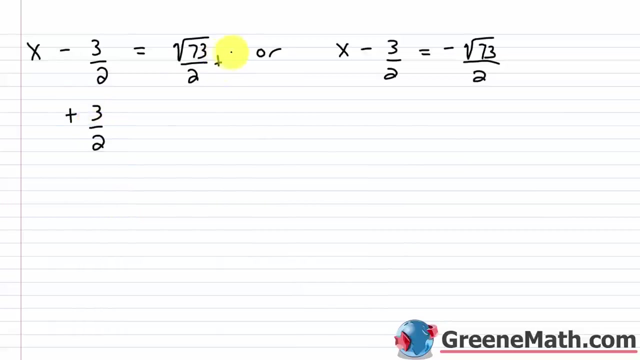 equal to plus or minus. Now I can split this up into the square root of 73 over the square root of four, which is two. So square root of 73 over two. So this is two different scenarios. I would have X minus three halves is equal to the square root of 73 over two. Then or X minus three halves is equal to the negative square root of 73 over two. All right. So the next thing I want to do is add three halves to both sides of the equation over here. So I will have X is equal to the square root of 73 plus three over two. Can't do anything else really here. That's kind of the best I can do. And then, or over here, I'm going to add three halves to both sides of the equation. And so I'm going to have X is equal to the negative square root of 73 plus three over two. 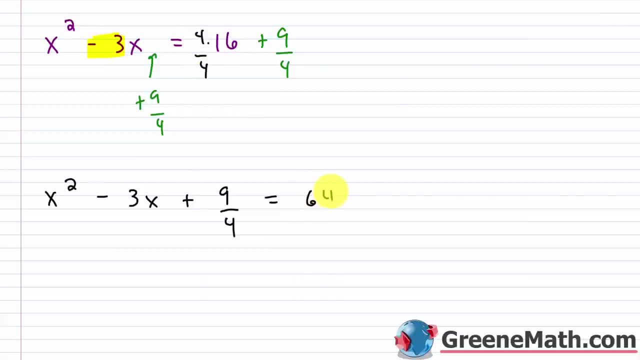 4 times 16.. 16 is of course, 64. So I'd have 64 plus 9 over 4.. And 64 plus 9 is 73. So this would be 73 fourths. Now, at this point, this is a perfect square trinomial. 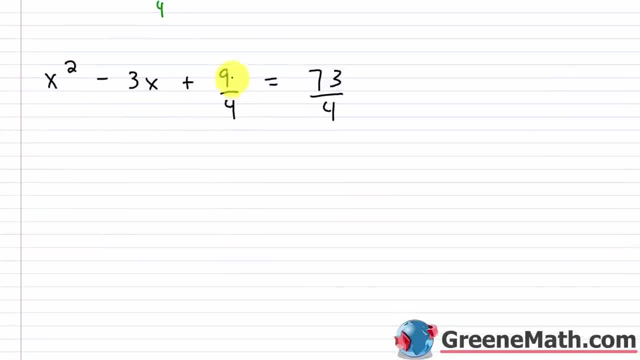 I can factor this, And I know a lot of you aren't used to seeing fractions when you go to factor stuff. It's not any more difficult. Just follow your pattern. So this is going to be x. You have a minus here. 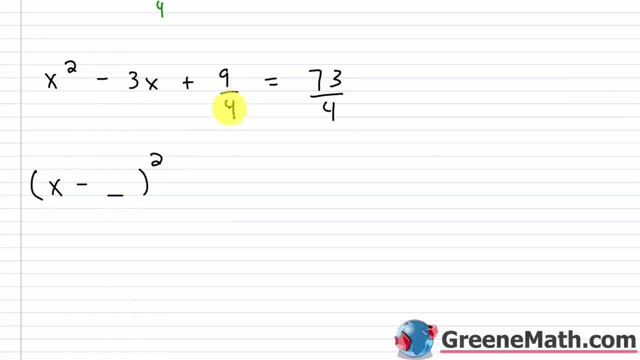 So this is minus. What's going to go in that position? Well, just take the square root of this. The square root of 9 is 3.. And the square root of 4 is 2.. So this is going to be 3 halves. 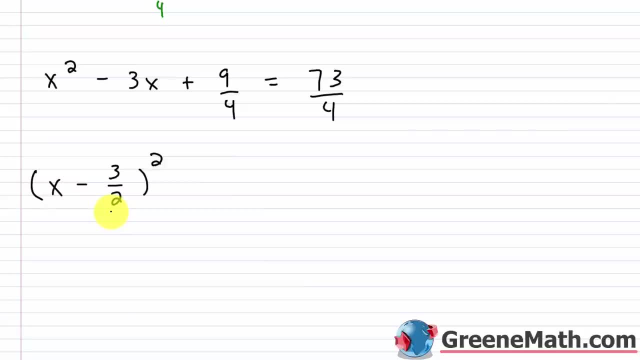 And go ahead and FOIL that out if you don't believe me. You're going to end up with x squared minus 3x plus 9 fourths. You're going to end up with x squared minus 3x plus 9 fourths. 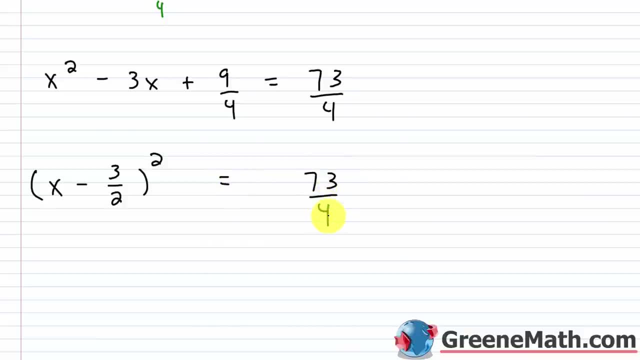 Okay, so this equals 73 fourths. Okay, so this equals 73 fourths, And now we use our square root property. So I take the square root of this side And then plus or minus the square root of this side. 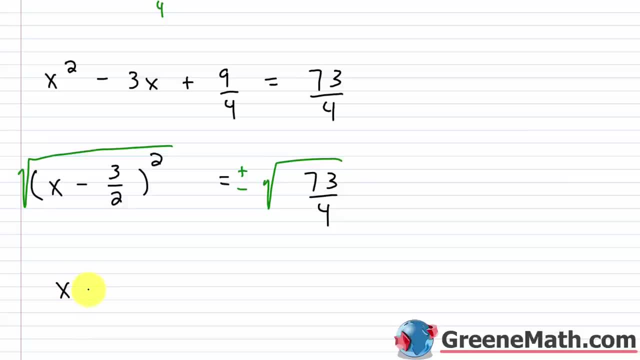 And what I'm going to end up with is x minus 3. halves is equal to plus or minus. Now I can split this up into the square root of 73 over the square root of 4, which is 2.. So the square root of 73 over 2.. 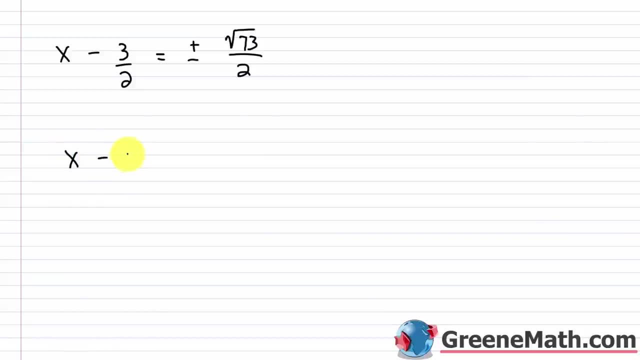 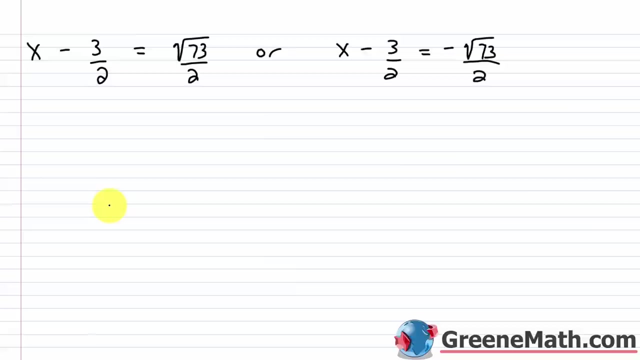 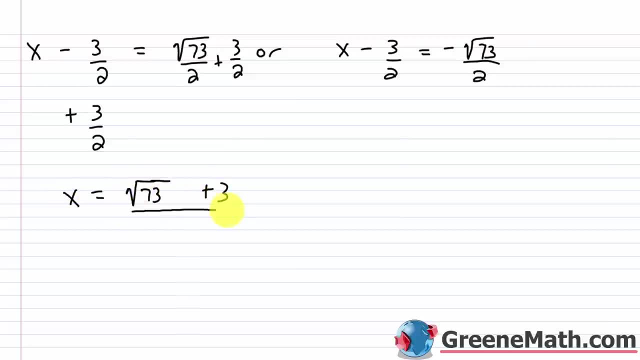 Then OR x minus 3 halves is equal to the negative square root of 73 over 2.. 3 plus 3 over 2, can't do anything else really here. that's kind of the best I can do. And then OR over- here I'm going to add 3 halves to both sides of the equation. 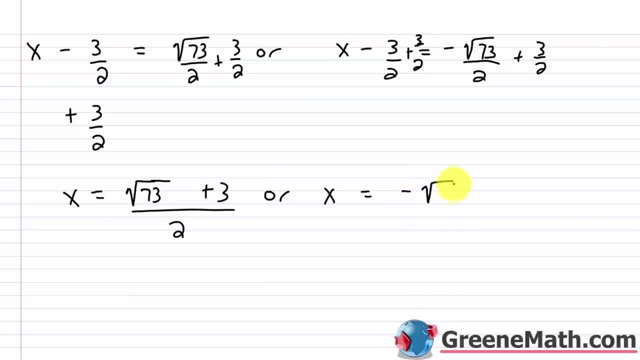 And so I'm going to have: x is equal to the negative square root of 73 plus 3 over 2.. So really I can condense this and say x is equal to plus or minus the square root of 73 plus 3 over 2.. 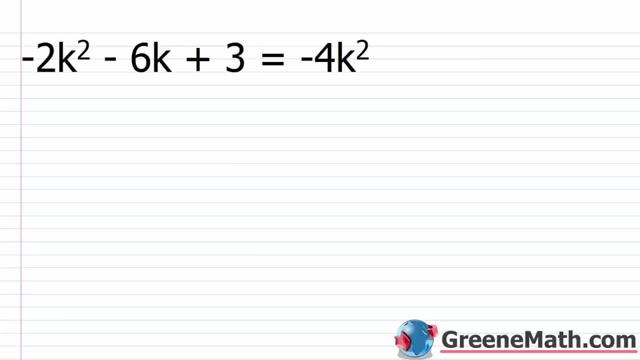 Alright, let's take a look at another one. So I have negative 2k squared minus 6k plus 3 is equal to negative 4k squared. So what I want to do? let me just add 4k squared to each side of the equation to start. 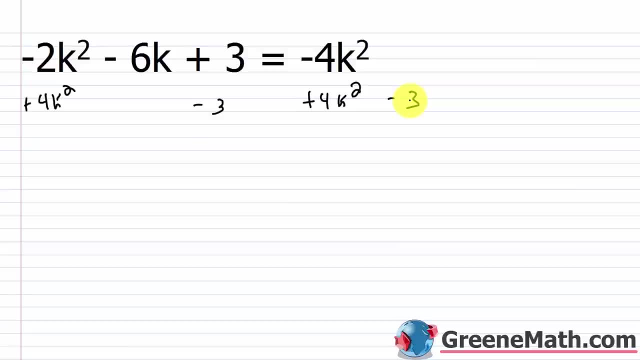 And let me subtract 3 away from each side of the equation. So negative: 2k squared plus 4k squared is 2k squared, Then minus 6k. this would cancel. so that's gone and this is equal to this would cancel. 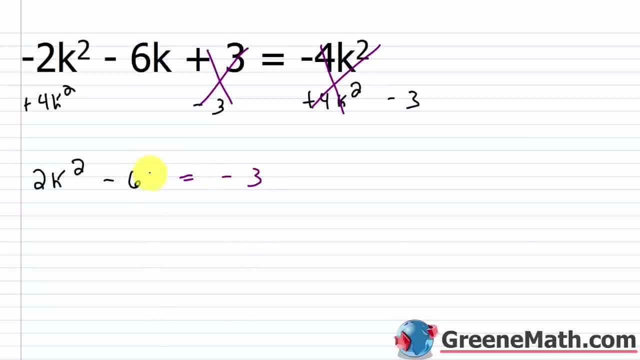 just negative 3.. So now we have a scenario that we haven't come across before. Notice that the coefficient on the squared term is a 2. So we don't want that. So the way we're going to get rid of it is we're going to divide both sides of the 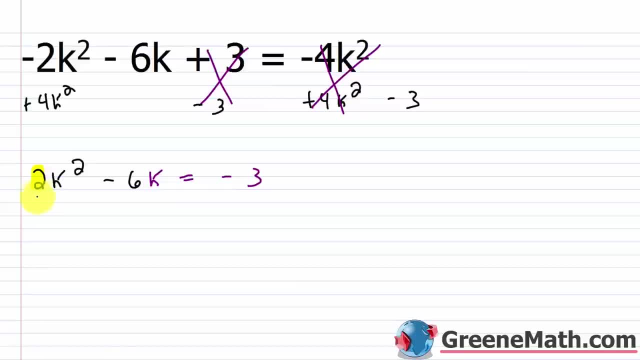 equation by 2.. So I divide this side of the equation by 2, and I divide this side of the equation by 2.. And what that's going to give me is you can just split this up and have 2k squared over. 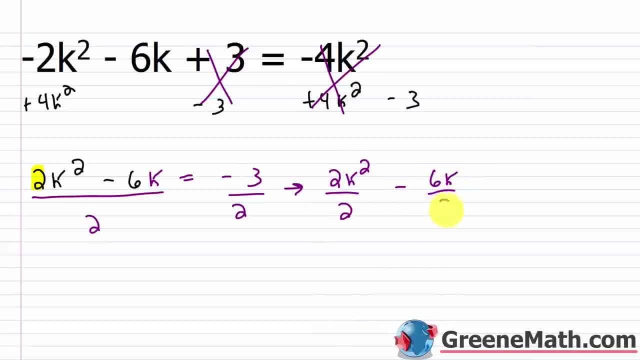 2 minus 6k over 2 is equal to negative 3 over 2.. And then we can see that this cancels with this and I just have k squared. So that's what I want. I want k squared. So the coefficient out here is a: 1 minus 6 over 2 is 3, so minus 3k is equal to negative. 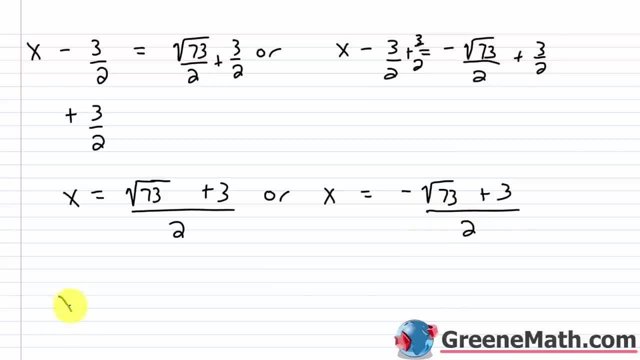 So really I can condense this and say X is equal to plus or minus the square root of 73 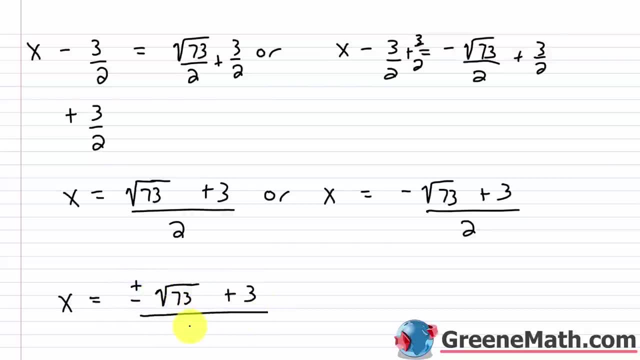 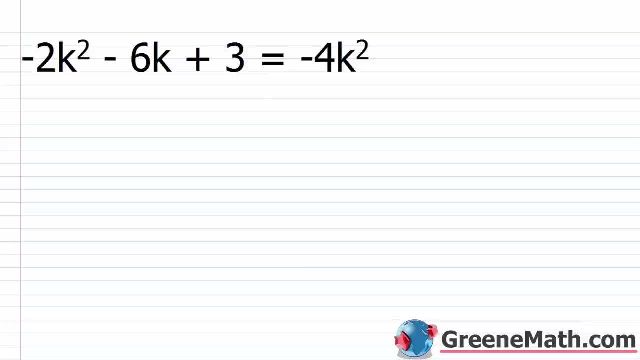 plus three over two. All right. Let's take a look at another one. So I have negative two K squared minus six K plus three is equal to negative four K squared. So what I want to do, let me just add four K squared to each side of the equation to start. And let me subtract the two halves. I'm going to subtract three away from each side of the equation. So negative two K squared plus four K squared is two K squared. Then minus six K. This would cancel. That's gone. And this is equal to, this would cancel just negative three. So now we have a scenario that we haven't come 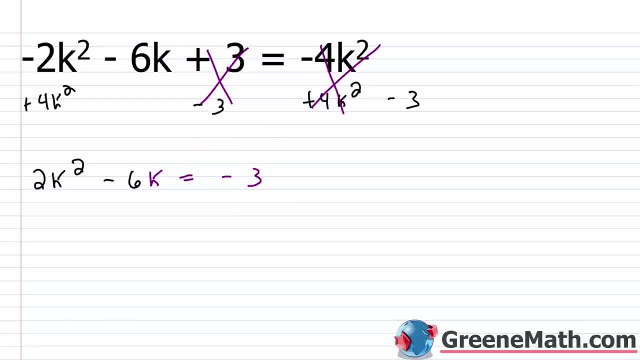 across before. Notice that the coefficient on the squared term is a two. So we don't want that. So 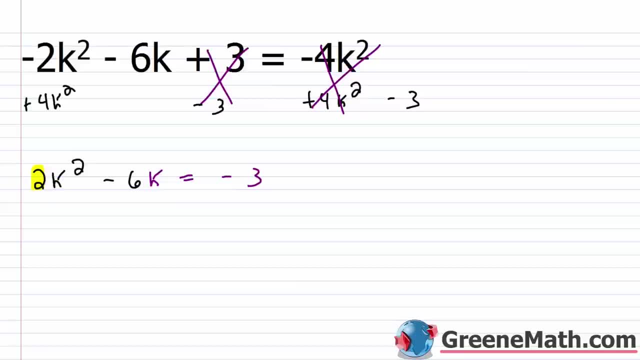 the way we're going to get rid of it, is we're going to divide both sides of the equation by two. So I divide this side of the equation by two and I divide this side of the equation by two. And what that's going to give me 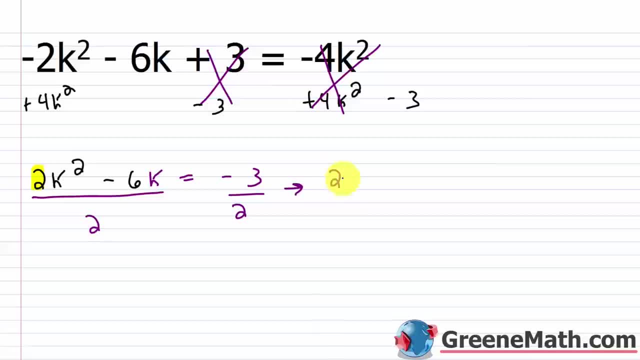 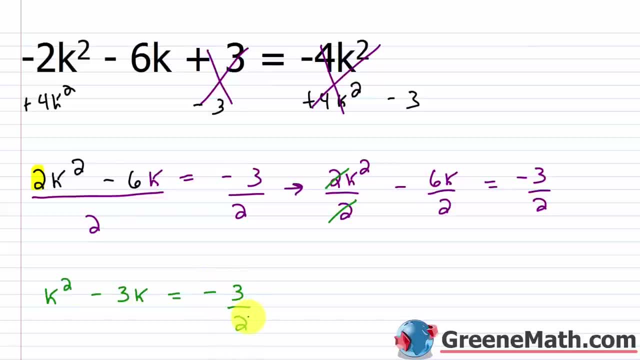 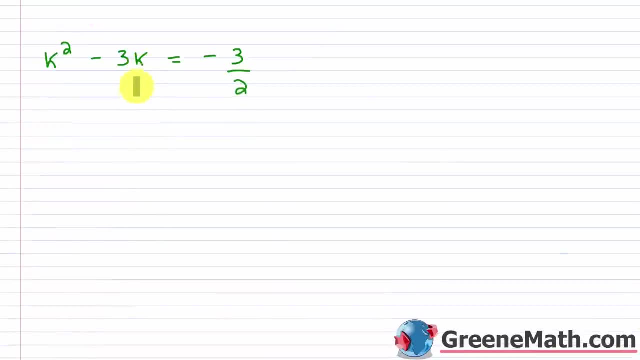 is equal to negative three halves. So now that I've done that, I want to get into completing the square. So I want to look at the coefficient for the variable raise to the first power. So that's negative three here. And I want to cut it in half. I want to cut it in half. So that means multiply by half. Speaker 1 So that means multiply by half. And then I'm going to use my formula here until the key Oooh and let me show how different each is. and then I want to square it, okay? So negative three times one half is negative three halves. 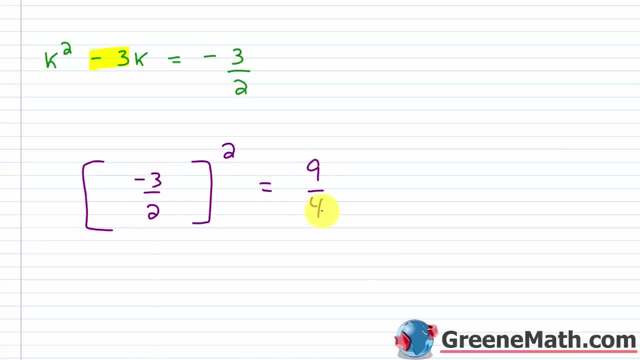 And if I square that, I get nine fourths, okay? Nine fourths. 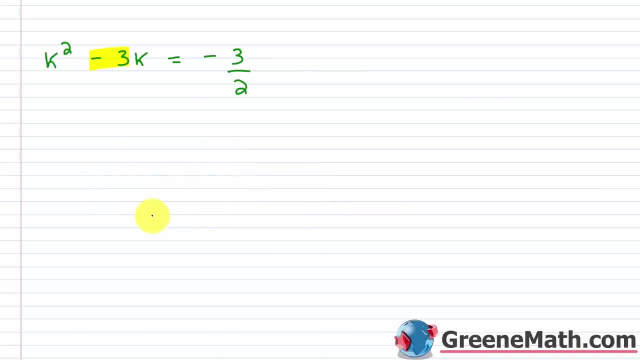 So I'm gonna add nine fourths to each side of this equation. 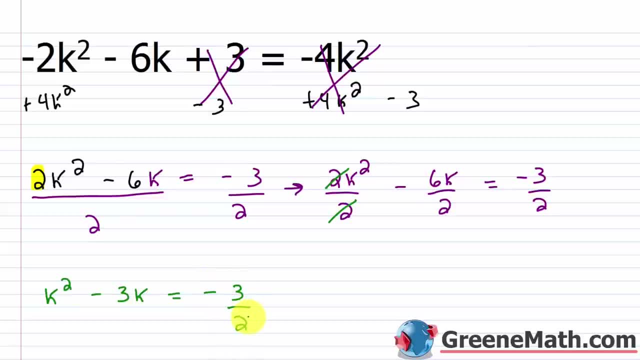 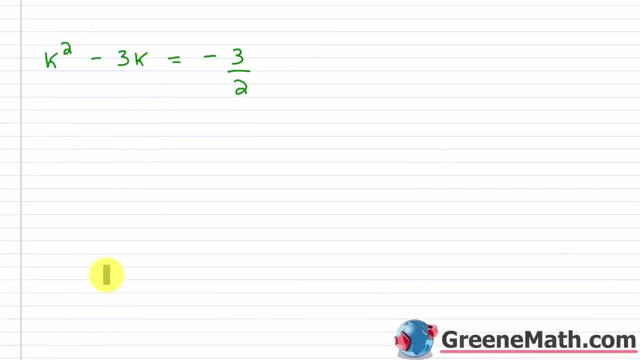 3 halves. So now that I've done that, I want to get into completing the square. So I want to look at the coefficient for the variable raised to the first power. So that's negative 3 here And I want to cut it in half. 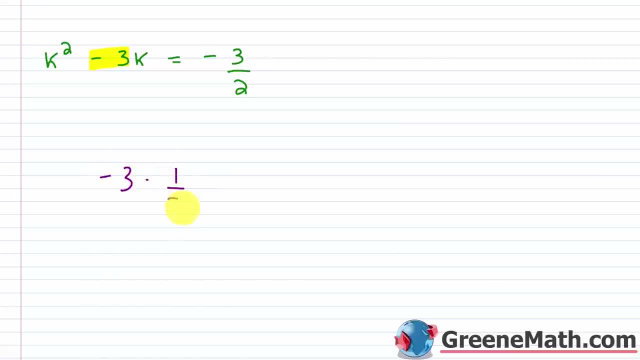 I want to cut it in half, So that means multiply by half. And then I want to subtract, I want to square it, So negative 3 times 1 half is negative 3 halves, And if I square that I get 9 fourths. 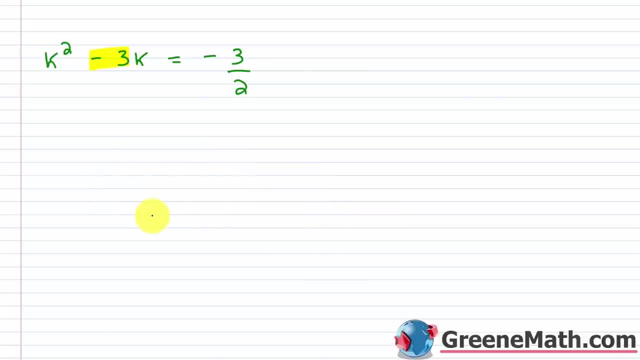 I'm going to add 9 fourths to each side of this equation, So I'll have k squared minus 3k plus 9 fourths is equal to negative 3 halves plus 9 fourths. OK, Okay. So over here on the right, I would get a common denominator going. Multiply this by 2 over. 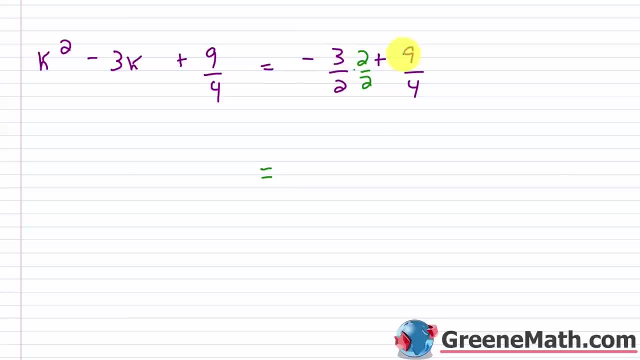 2. And I'm going to have negative 6 plus 9,, which is 3, over 4.. This is 3 fourths Over. here I'm going to go ahead and factor this. This is a perfect square trinomial now. So I'm going to. 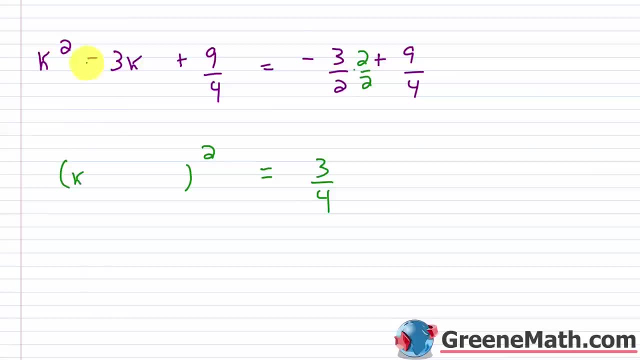 factor this into: I have k, I have minus. and then what's the square root of 9 fourths? Well, we know it's 3 halves. So I get k minus 3 halves. That quantity is squared and this equals 3. 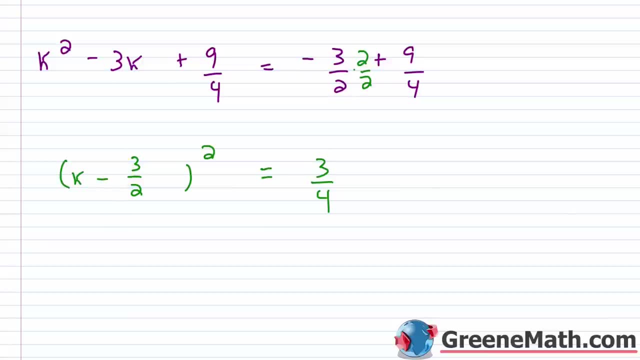 fourths. So now I can use my square root property, take the square root of this side and then plus or minus the square root of this side, And I'll end up with k minus 3 halves, because this would cancel with this, And this is equal to plus or minus the square root of 3 fourths. 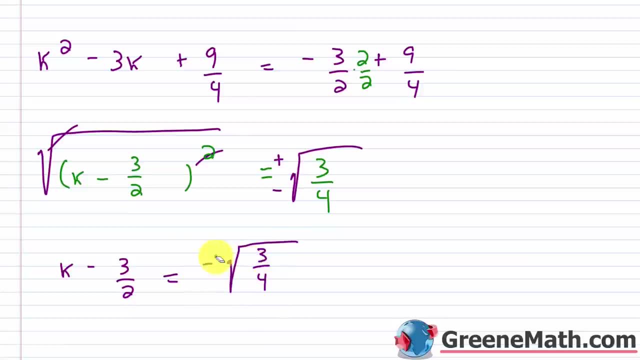 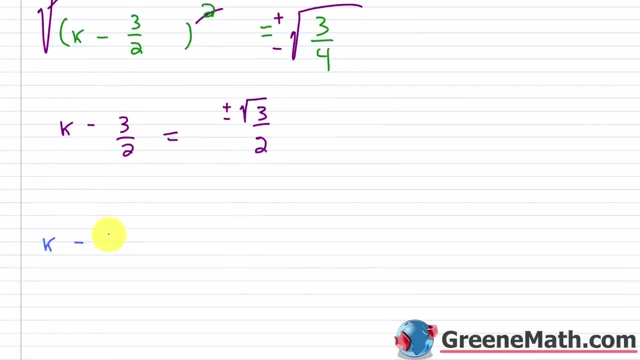 Now, Now the square root of 4 is 2, so really I could rewrite this as plus or minus the square root of 3 over 2.. So let's scroll down and we'll look at these two scenarios. So we'll have k minus 3 halves is equal to square root of 3 over 2, or we'll also see: 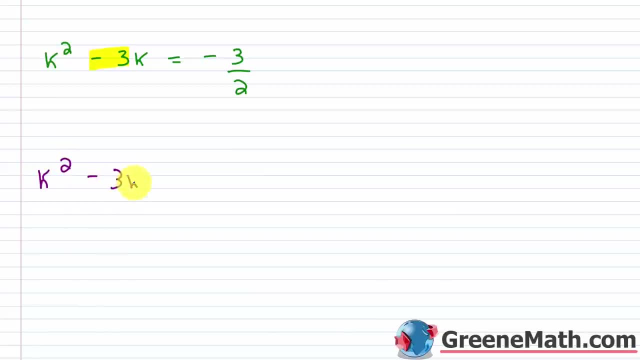 So I'll have k squared minus three k plus nine fourths is equal to negative three halves plus nine fourths. 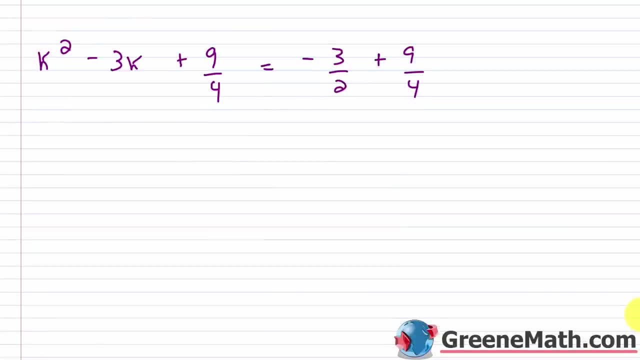 Okay, so over here on the right, I would get a common denominator going. Multiply this by two over two, and I'm gonna have negative six plus nine, which is three, over four. This is three fourths. 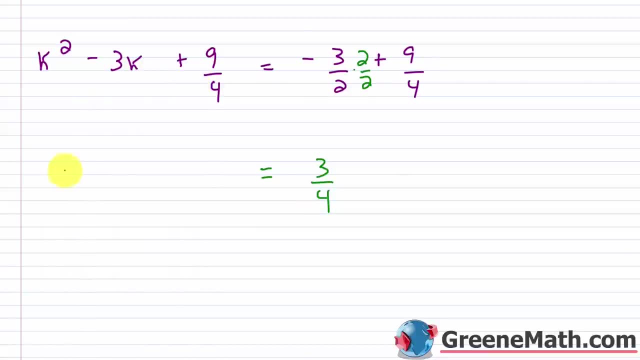 Over here, I'm gonna go ahead and factor this. This is a perfect square trinomial now. So I'm gonna factor this into, I have k, I have minus, and then what's the square root of nine fourths? Well, we know it's three halves. 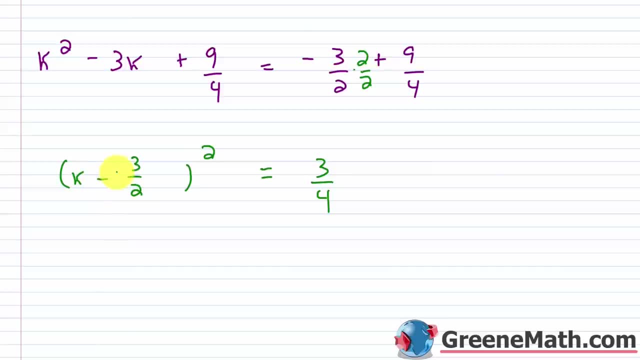 So I get k minus three halves. That quantity is squared, and this equals three fourths. 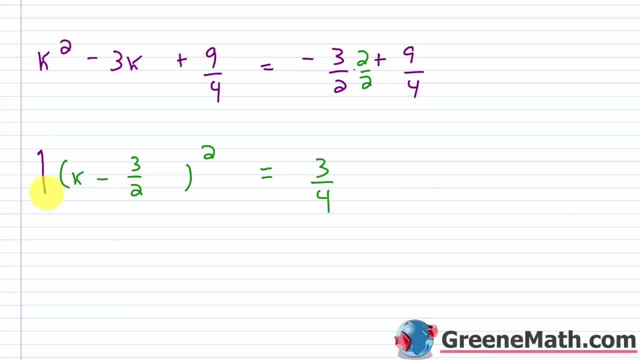 So now, I can use my square root property, take the square root of this side, and then plus or minus the square root of this side, and I'll end up with k minus three halves, right, because this would cancel with this, and this is equal to plus or minus the square root of three fourths. Now, the square root of four is two, so really, I could rewrite this as plus or minus the square root of three over two. 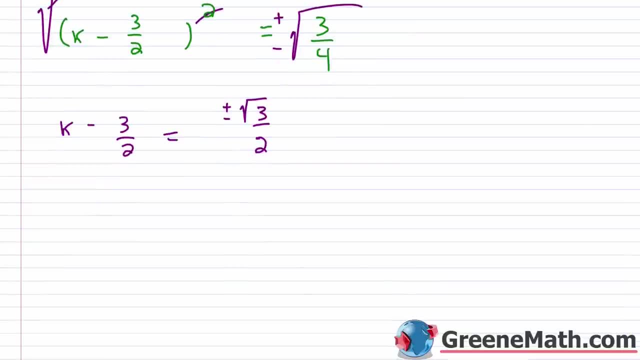 So let's scroll down, and we'll look at these two scenarios. 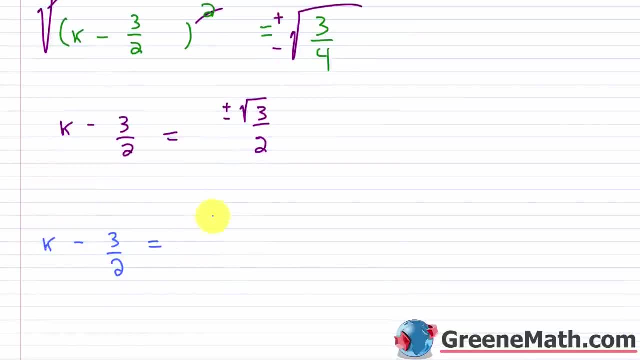 So we'll have k minus three halves is equal to square root of three over two, 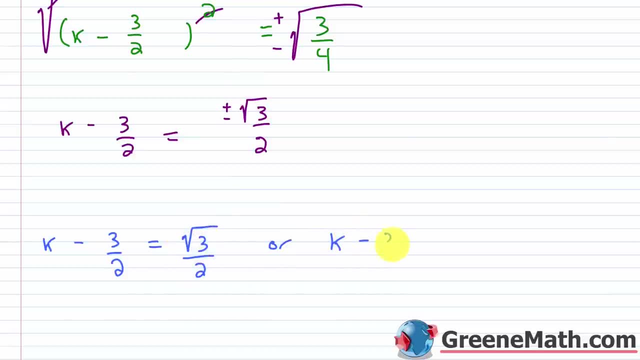 or we'll also see k minus three halves is equal to the negative square root of three over two. 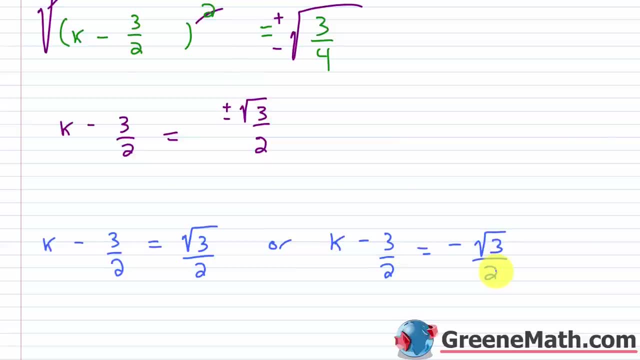 So in each scenario, to isolate k, I'm gonna be adding three halves to each side of the equation. 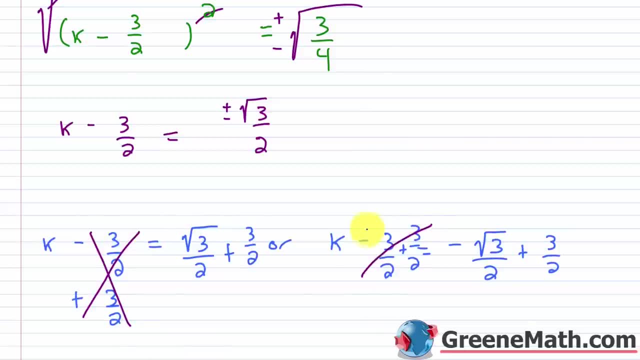 And what's gonna happen is this is gonna cancel, and this is gonna cancel, and what I'm gonna be left with is k is equal to 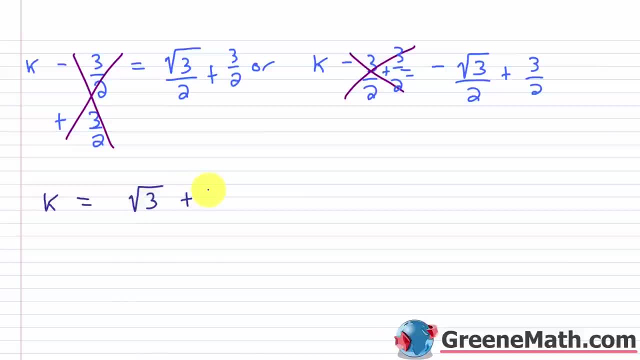 the square root of three plus three over that common denominator of two, or we could say k is equal to the negative square root of three plus three over the common denominator of two, or you could say k is equal to plus or minus the square root of three plus three all over two. 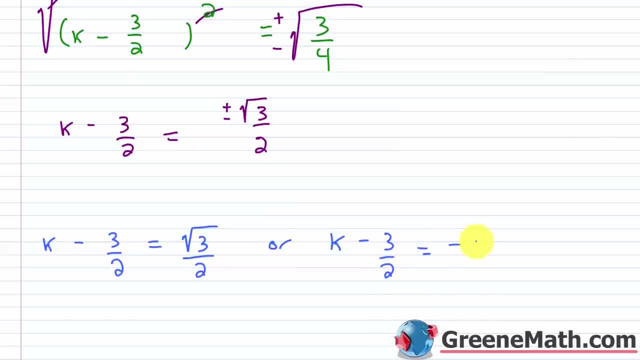 k minus 3 halves is equal to the negative square root of 3 over 2.. So in each scenario to isolate k, I'm going to be adding 3 halves to each side of the equation And what's going to happen is this is going to cancel and this is going to cancel. 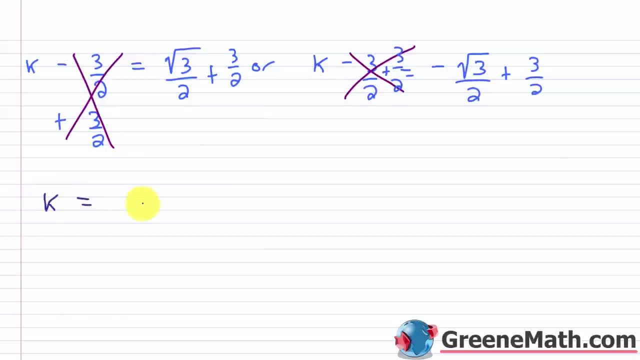 And what I'm going to be left with is k is equal to the square root of 3 over 2.. So I'm going to have k minus square root of 3 plus 3 over that common denominator of 2, or we could say k is equal to the negative square root of 3 plus 3 over the common denominator. 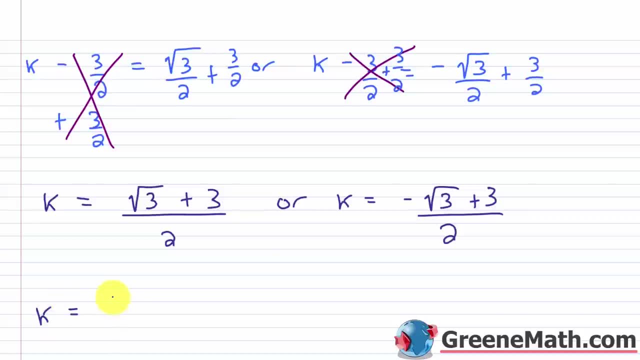 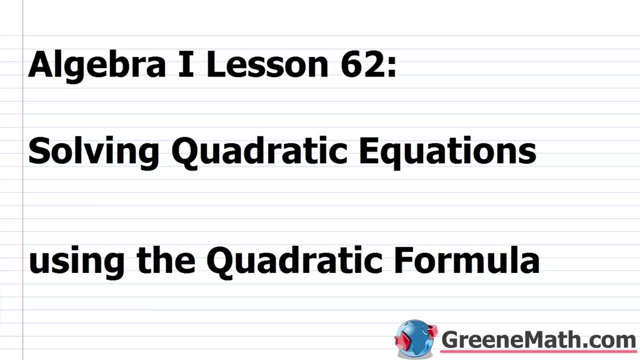 of 2, or I could say k is equal to, plus or minus, the square root of 3 plus 3, all over 2.. Hello and welcome to Algebra 1, Lesson 62.. In this video we're going to learn about square root of 3 over 2.. 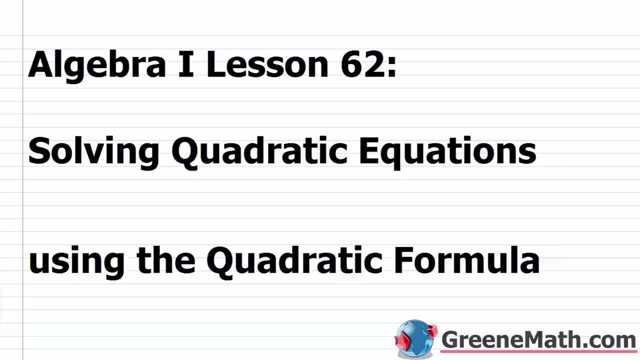 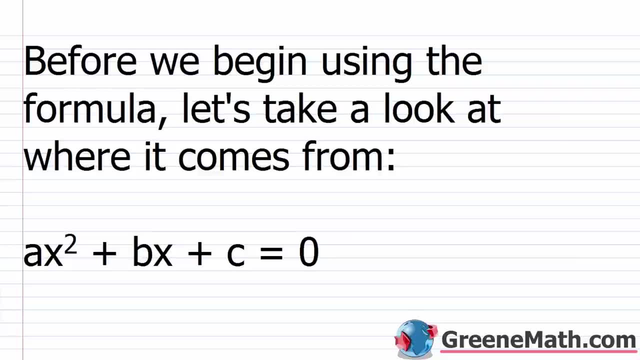 Let's get started. Let's start by solving quadratic equations using the quadratic formula. So when we first started learning about quadratic equations, we only dealt with quadratic equations that we could solve via factoring, And we kept it that way for a while, and then, in the last lesson, we learned how to solve. 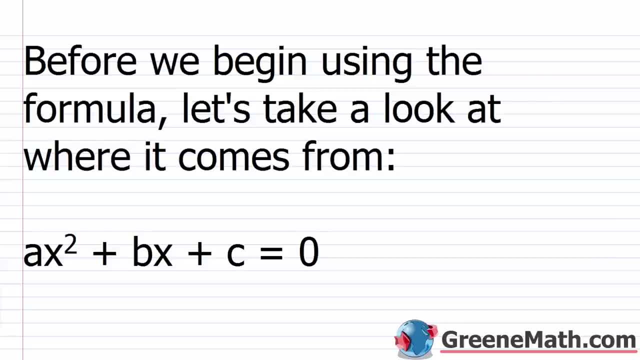 a quadratic equation, whether we could factor it or not using a process known as completing the square. Now, completing the square is one of those things where it's very, very tedious and there's so many things to do, So there's so many steps involved. it's very easy to make a mistake. 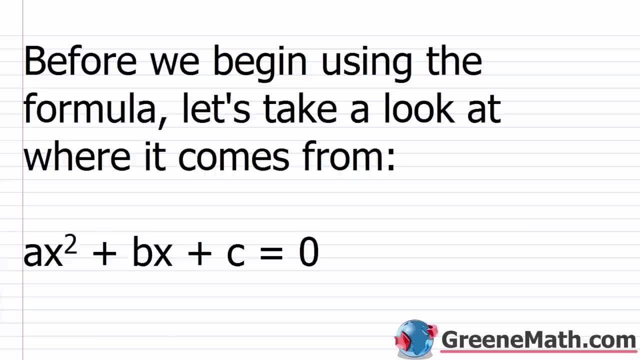 So in this lesson we're going to look at an easier process to solve any quadratic equation that you're going to come across. So this is known as solving a quadratic equation using the quadratic formula. But before we begin using the formula, let's take a look at where it actually comes from. 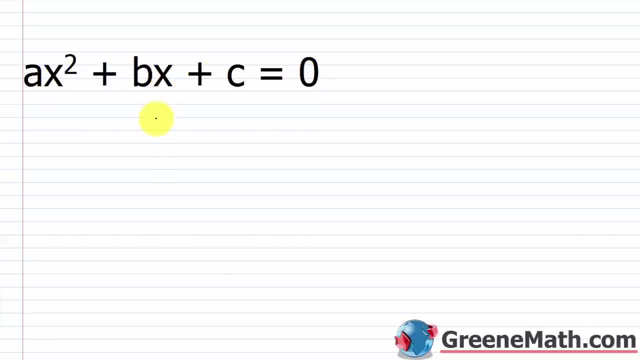 So we see ax squared plus bx plus c equals 0.. This is standard 4.. And of course this is a generic example. All I'm looking at here is I have my squared variable first, my variable to the first, power second and then my constant third. 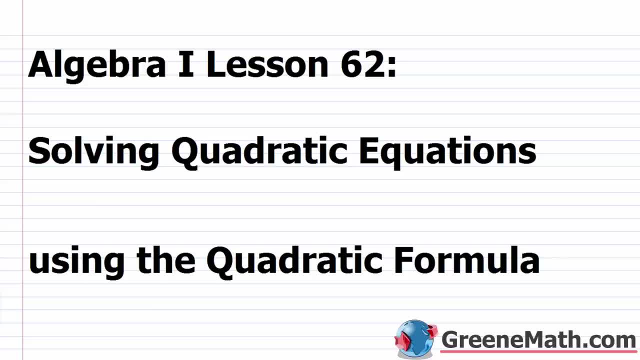 Hello, and welcome to algebra 1 lesson 62. In this video, we're gonna learn about solving quadratic equations using the quadratic formula. 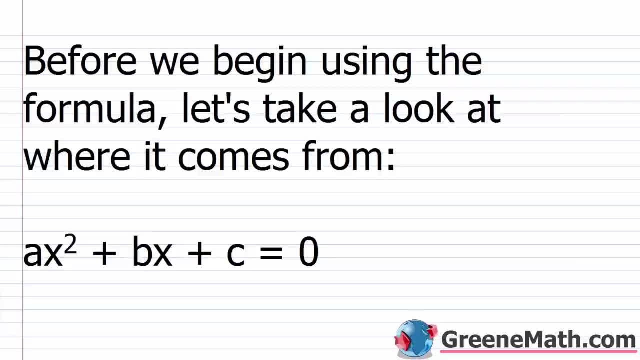 So when we first started learning to solve equations, it was pretty easy. 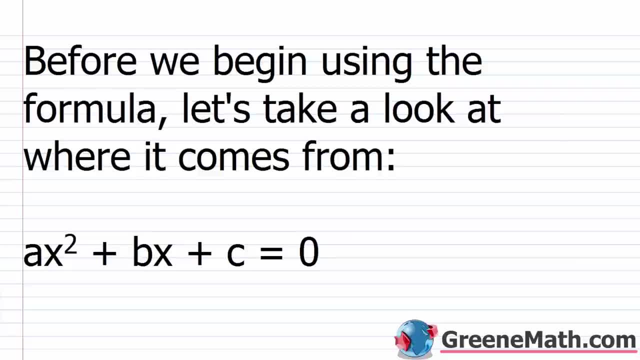 learning about quadratic equations we only dealt with quadratic equations that we could solve via factoring and we kept it that way for a while and then in the 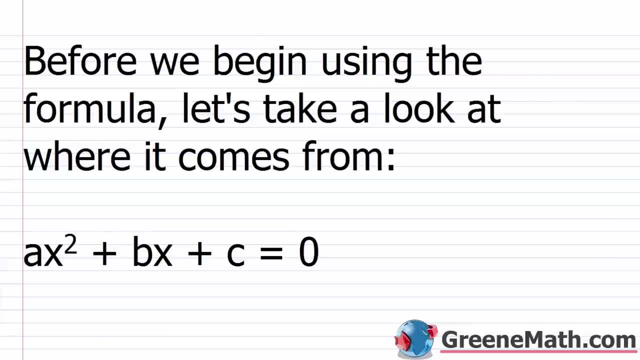 last lesson we learned how to solve a quadratic equation whether we could factor it or not using a process known as completing the square now completing 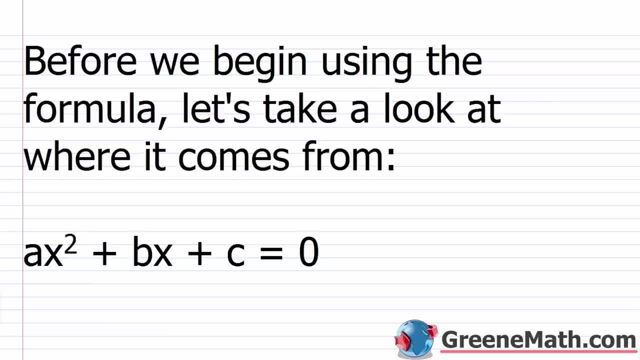 the square is one of those things where it's it's very very tedious and there's so many steps involved it's it's very easy to make a mistake so in this lesson 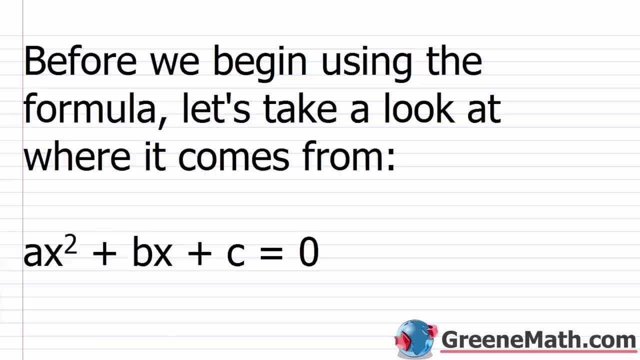 we're going to look at an easier process to solve any quadratic equation that you're going to come across so this is known as solving a quadratic equation using the quadratic formula but before we begin using the formula let's take a 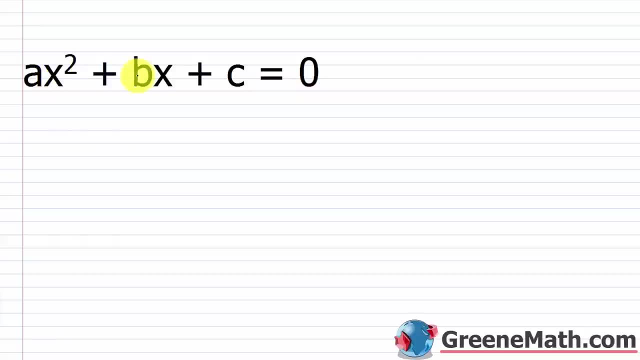 look at where it actually comes from so we see ax squared plus B X plus C equals 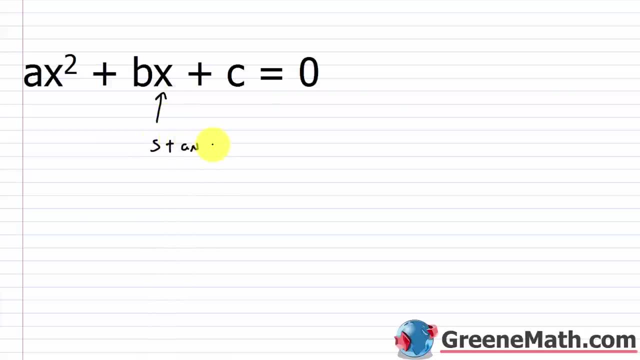 0 this is standard 4 and of course this is a generic example all I'm looking at is a generic example all I'm looking at is a generic example all I'm looking at 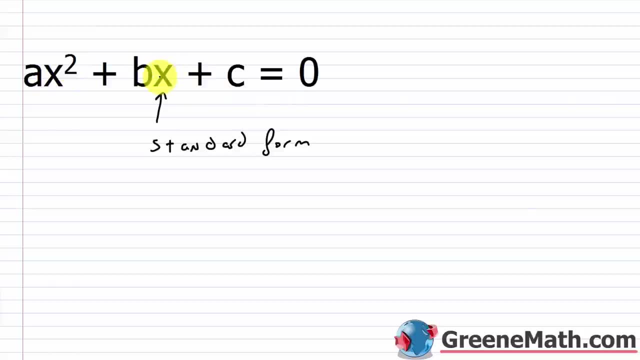 here is I have my squared variable first my variable to the first power second and then my constant third so I could have something like 6x squared plus 2x minus 7 equals 0 it's a standard form and one of the things we're gonna have to do is match things up so in other words this right here the coefficient for x squared that's a this 2 right here the coefficient for X to the first power that's B this negative 7 is going to be C or the constant term and it's very important that you include the sign with this because remember I could write this as a plus and then a negative 7 okay so that C there is negative 7 and the variable does not have to be X again that's just a generic example you can see something like 3m 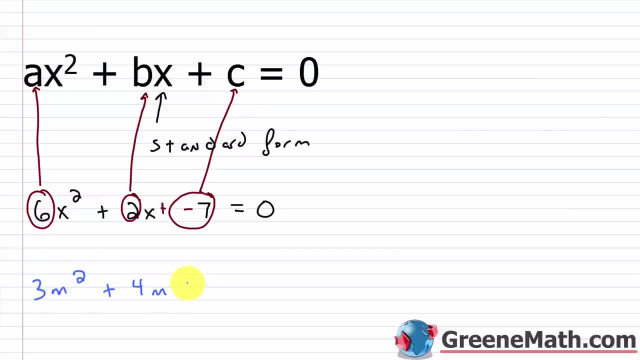 squared plus 4m minus 2 equals 0 now you have 3 is the coefficient for M squared 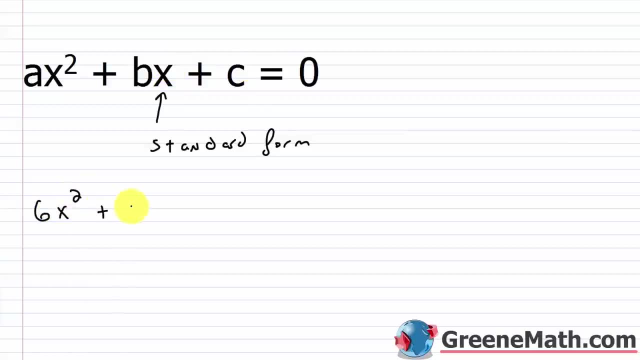 So I could have something like: 6x squared plus 2x minus 7 equals 0.. This is standard 4. And one of the things we're going to have to do is match things up. So, in other words, this right here: the coefficient for x squared, that's a, This 2, right here. 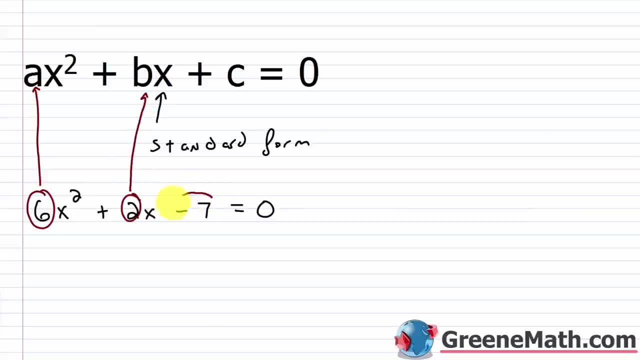 the coefficient for x to the first power, that's b. this negative 7 is going to be c or the constant term, and it's very important that you include the sign with this because, remember, i could write this as a plus and then a negative 7. okay, so that c, there is negative 7 and the variable does not. 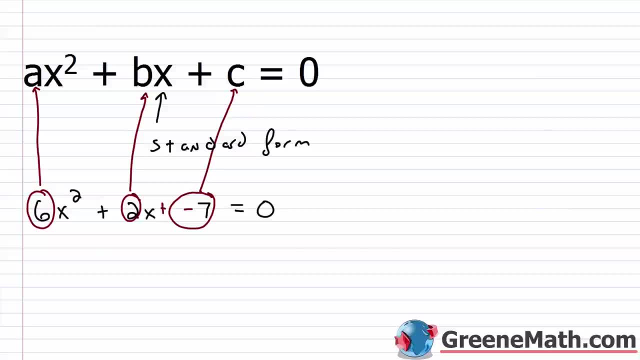 have to be x again. that's just a generic example. you could see something like: 3m squared plus 4m minus 2 equals 0. now you have 3 as the coefficient for m squared. so 3 is a, 4 is the coefficient for. 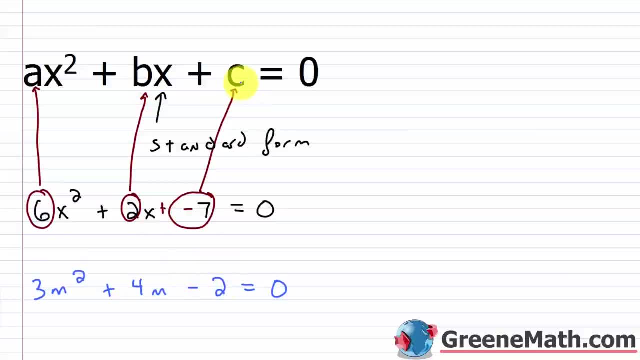 m to the first power. so 4 is b and then negative 2 would be c. that's your constant. now let me erase this real quick and i want to show you how to derive the quadratic formula. and after that we're going to look at some examples using the quadratic formula and you do a few examples of that and 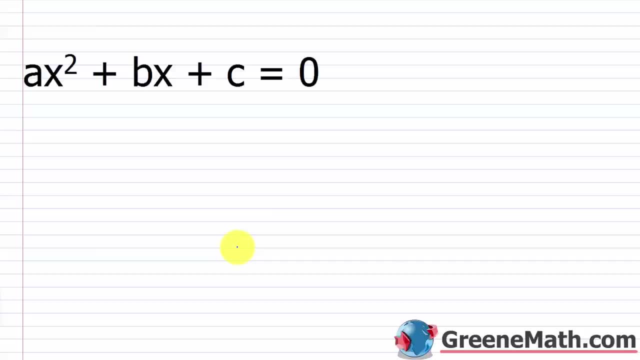 basically you're good to go right. you're just plugging things in as long as you can do some basic formulas, and then you're good to go. so let's go ahead and start with this equation. so you can do some basic formulas and you do a few examples of that and basically you're good to go. 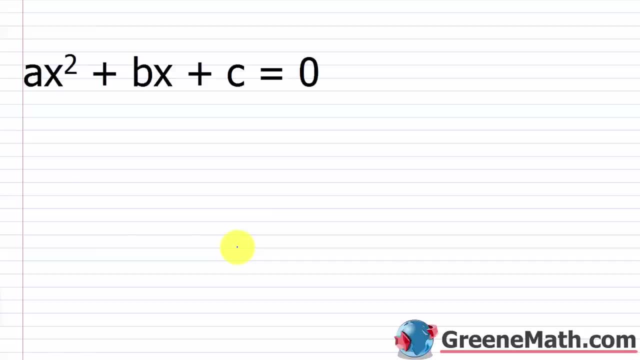 arithmetic, you're good to go. so for this guy right here, ax squared plus BX plus C equals zero. what is the solution? and I realize we don't have numbers. we have an a, a B and a C that represent numbers. but how would I get a solution? well, we know. 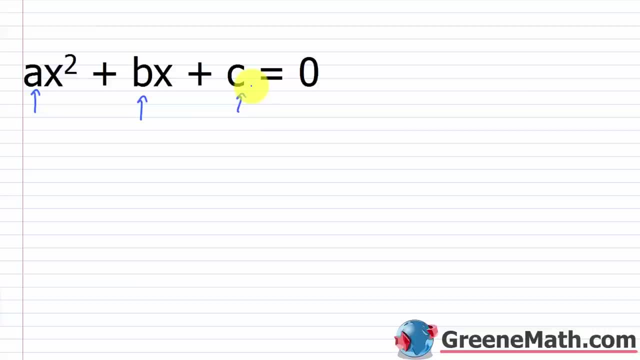 already that we can use completing the square, so let's go ahead and do that. let's start out by doing one. let's just copy this: ax squared plus BX plus C equals zero. I know I want all the variable terms on one side. these are the variable terms and I want my constant on the other, so I got to move that over. so 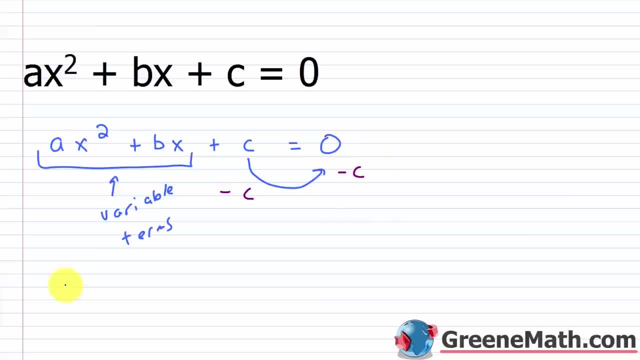 how to do that. again, I just subtract C away from each side of the equation, so I would have: ax squared plus BX is equal to negative C. right, this is going to cancel. so once I've done that, the next thing that I've told you is that you're going to have to do. is you're going to have to do? is you're going to? so 3 is 0. 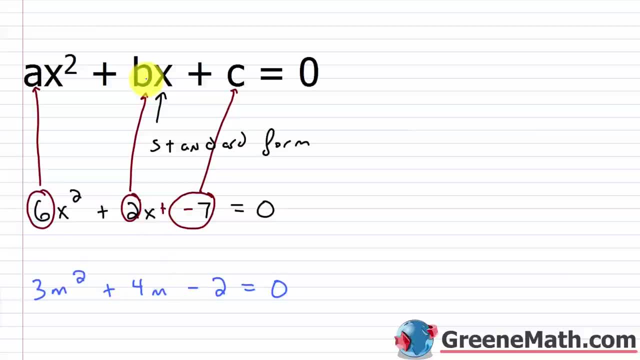 a, four is the coefficient for m to the first power, so four is b, and then negative two would be c. That's your constant. Now, let me erase this real quick, and I want to show you how to derive the quadratic formula. And after that, we're going to look at some examples using the quadratic formula, and you do a few examples of that, and basically you're good to go, right? You're just plugging things in. As long as you can do some basic arithmetic, you're good to go. So for this guy right here, ax squared plus bx plus c equals zero, what is the solution? And I realize we don't have numbers. We have an a, a b, and a c that represent numbers, but how would I get a solution? 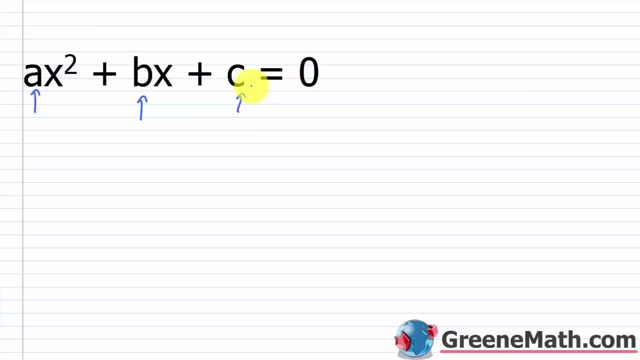 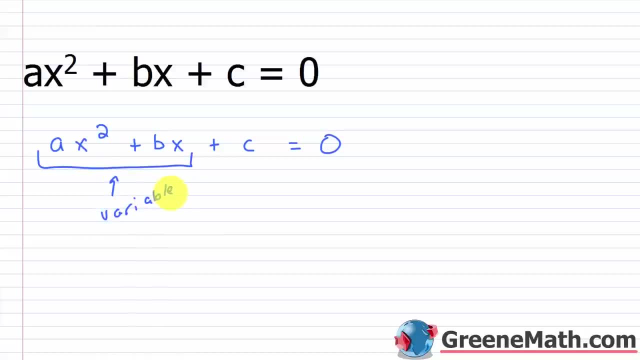 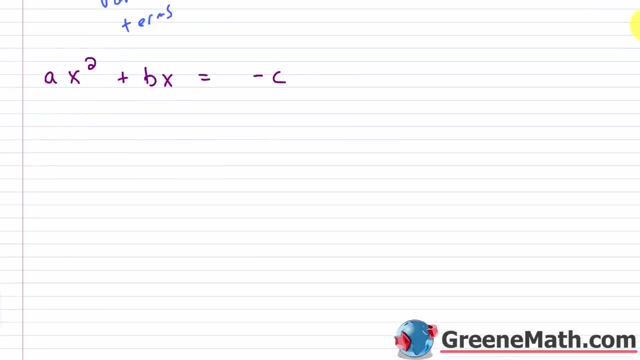 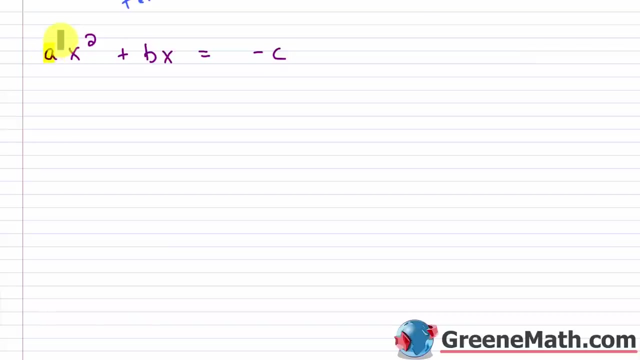 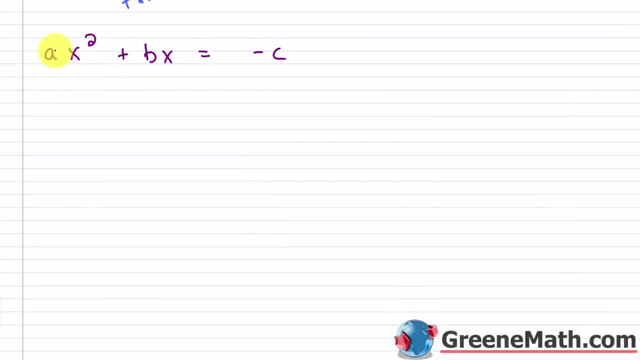 that you always want the coefficient out here to be a 1. now, when you use a generic example like this, you have a that represents your coefficient. a could be one. it could really be any number that you choose. it just can't be zero. because if I had a 0 here, let's say I put zero there, zero times X, square to. 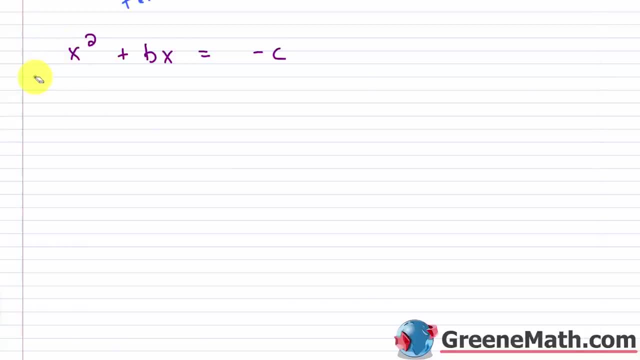 zero, you no longer have a quadratic equation. so actually that's one restriction: that you have a quadratic equation- your a or your coefficient for variable cannot be zero. Right now a can be anything other than zero. So to deal with that, we're going to get rid of a from right there, And I do that with some basic algebra. I divide. 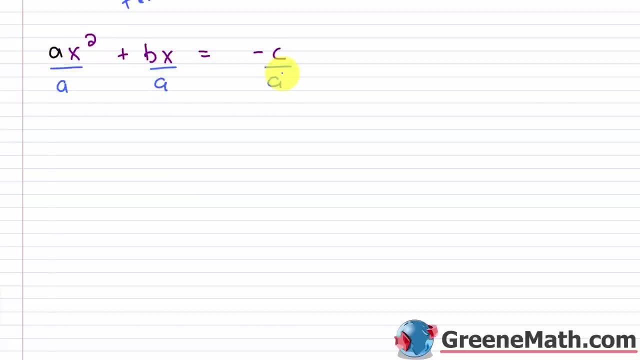 both sides of the equation by a, And what happens is it's going to cancel here And now. the coefficient for x squared is definitely one. So I have x squared plus b over a times x is equal to negative c over a. So the next step is the one that everybody struggles with. We're going to 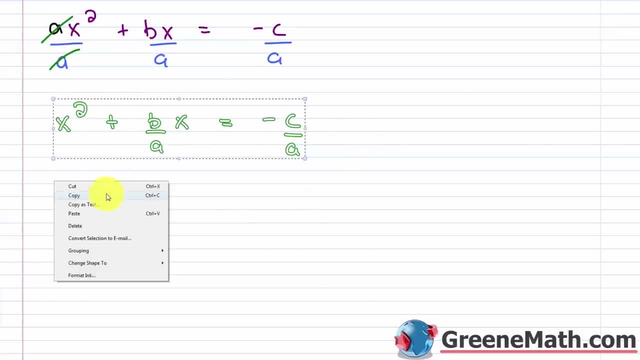 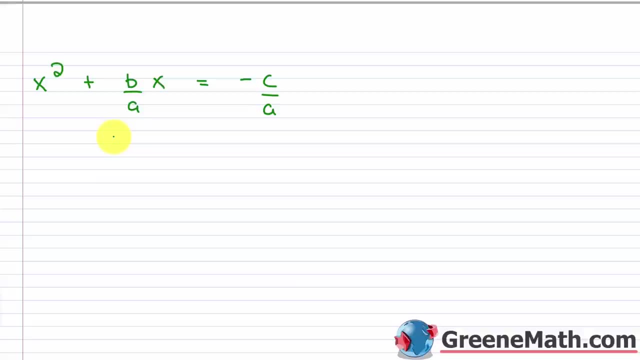 complete the square. Let me just copy this real quick. I'm going to move it down. I have some room And to complete the square I take one half of the coefficient of the first degree term and I square it And then I'm going to add that to both sides. So this is the coefficient for. 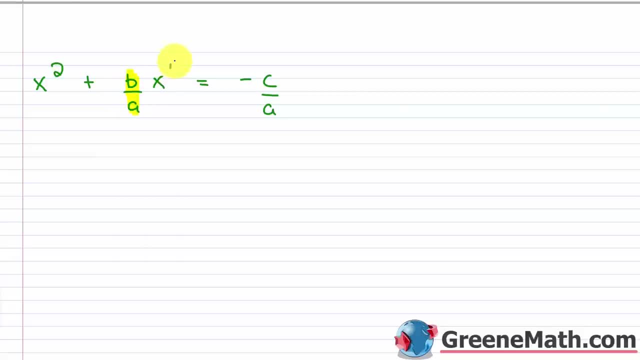 the first degree term. This is x to the first power And this is your coefficient. And again, when we work with kind of generic examples it's hard to see them right. But this is your variable here. x is the variable, b over a is the coefficient. So I want to cut it in half. 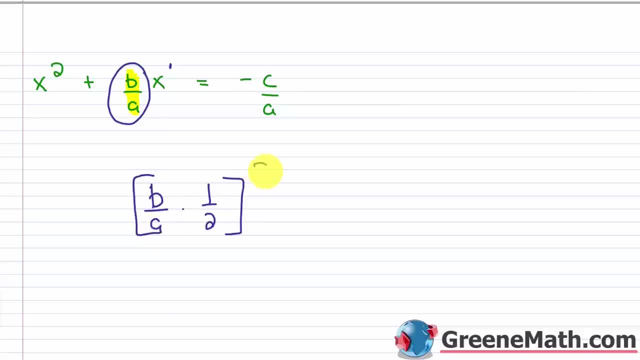 So multiply it by half And then I want to square it. So this would be b over 2a, b over 2a, And if I square that, b squared is b squared, And then 2 squared is 4.. a squared is a squared. 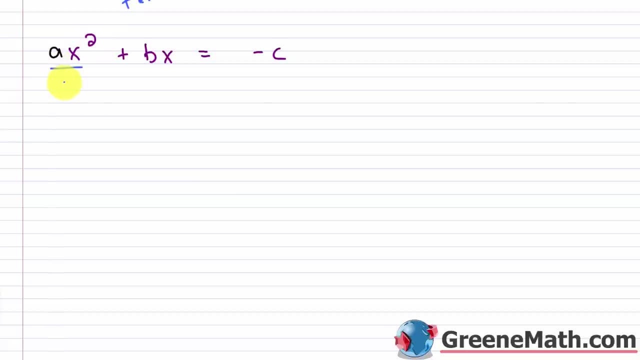 And I do that with some basic algebra, I divide both sides of the equation by a. And what happens is it's going to cancel here. And now the coefficient for x squared is definitely one. So I have x squared, plus b over a times x is equal to negative c over a. So the next step is the one 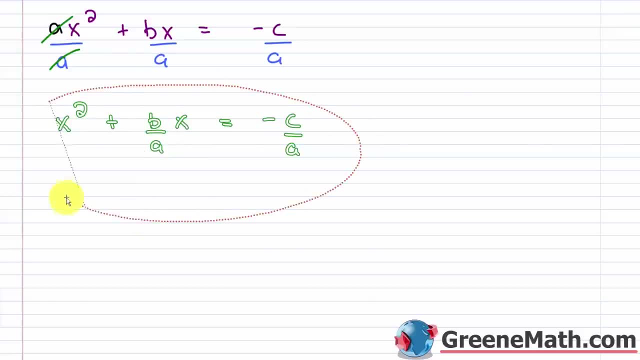 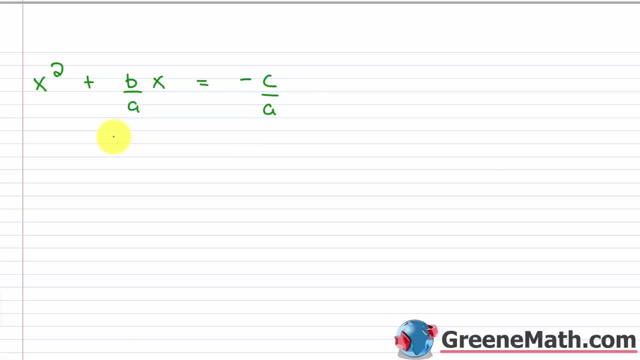 that we're going to complete the square. Let me just copy this real quick, I'm going to move it down. I have some room. And to complete the square, I take one half of the coefficient of the first degree term. And I square it, okay, and then I'm going to add that to both sides. So this is the coefficient for the first degree term. This is x to the first power. And this is your coefficient. And again, when we work with kind of generic examples, it's hard to see them, right? But this is your variable, you're going to be able to see it. But you're going to be able to see it. So you're here. X is the variable, b over a is the coefficient. So I want to cut it in half, so multiply it by half, and then I want to square it. So this would be b over 2a, b over 2a, and if I square that, b squared is b squared, and then 2 squared is 4, a squared is a squared. 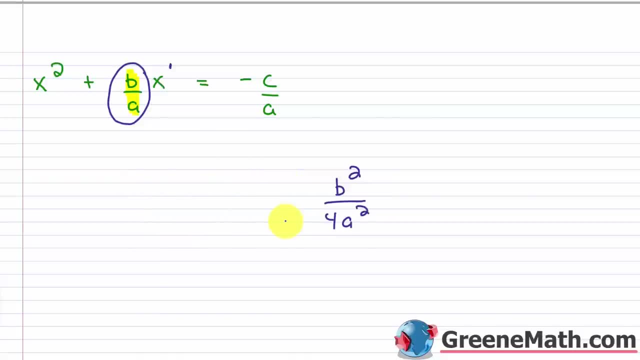 So this is the value that I'm going to add to each side of the equation. So let me just kind of slide this down. And so I'm going to add b squared over 4a squared to both sides of the equation. Now on the right side of the equation, I want to get a common denominator going. So how can I do that? Well here I have 4a squared, here I just have a. So if I multiplied by 4a, top and bottom here, I would get, let me kind of do this down here, b squared minus 4a times c is 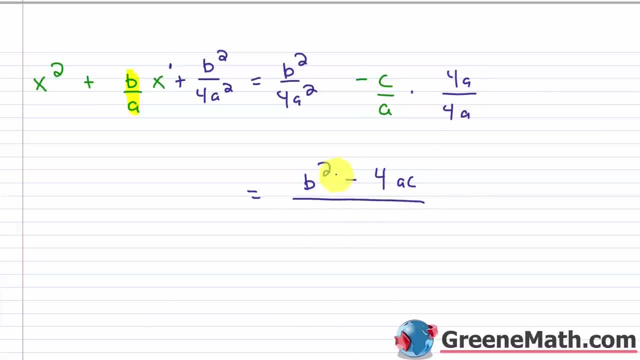 4ac, all over, this would now be a common denominator of 4a squared. Okay, so the right side, that's good to go. So now the left side is a perfect square trinomial. So we're going to 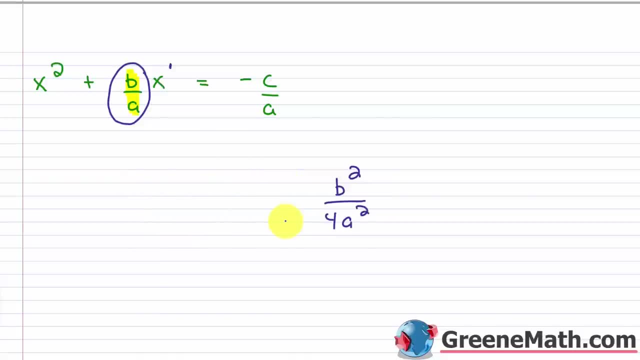 So this is the value that I'm going to get, And then I'm going to multiply it by a squared, And then I'm going to add to each side of the equation. So let me just kind of slide this down. And so I'm going to add b squared over 4a squared, to both sides of the equation. 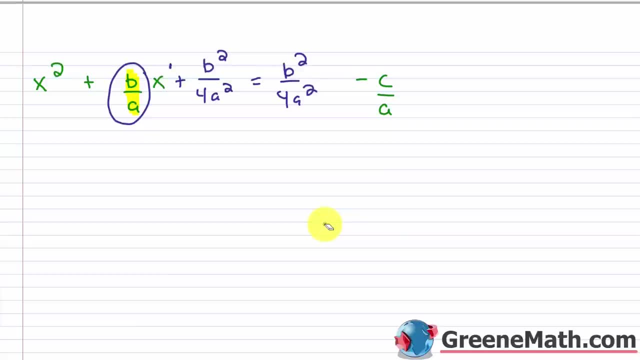 Now, on the right side of the equation, I want to get a common denominator going. So how can I do that? Well, here I have 4a squared, Here I just have a. So if I multiply I get a common denominator. And then I'm going to add b squared over 4a squared. 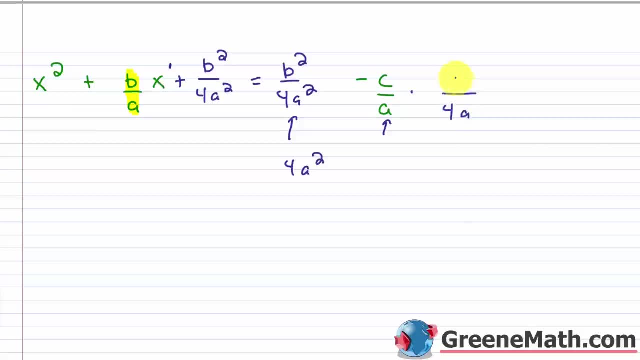 So if I multiply by 4a top and bottom here, I would get- let me kind of do this down here- b squared minus 4a times c is 4ac all over. this would now be a common denominator of 4a squared. 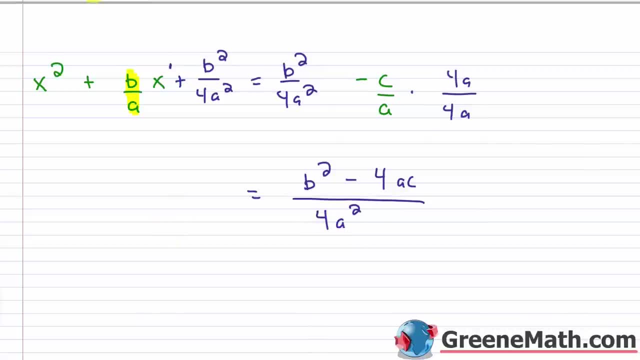 Okay, so the right side, that's good to go. So now the left side is a perfect square trinomial. So we're going to factor this guy. We know the first position would be x, And then there's a plus there, And then in this position the square root of b squared is b. 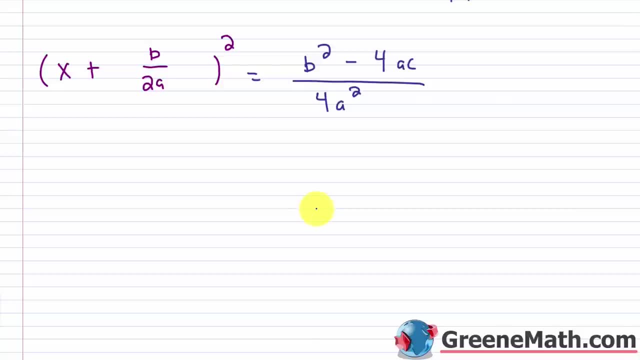 The square root of 4a. squared is 2a. So now what I want to do is use my square root property. Let me take the square root of this side and I'm going to go plus or minus the square root of this side. 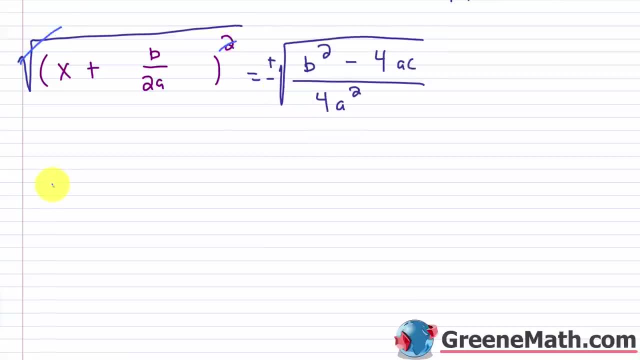 And of course this is going to cancel with this And I'm going to have: x plus b over 2a is equal to plus or minus, the square root of b squared minus 4ac over 4a squared. All right, let's scroll down. 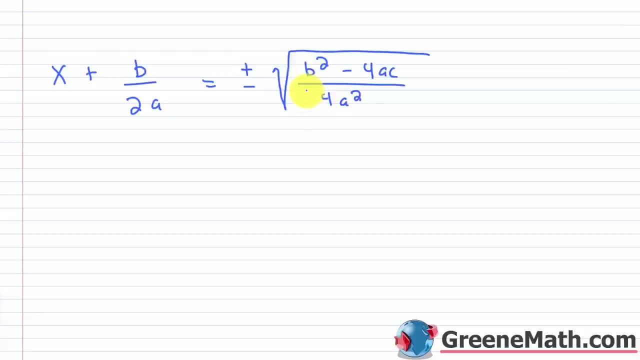 And one of the things we can do is we can break this up right. I know if I have the square root of, let's say, 1. fourth, this is equal to the square root of 1 over the square root of 4,. 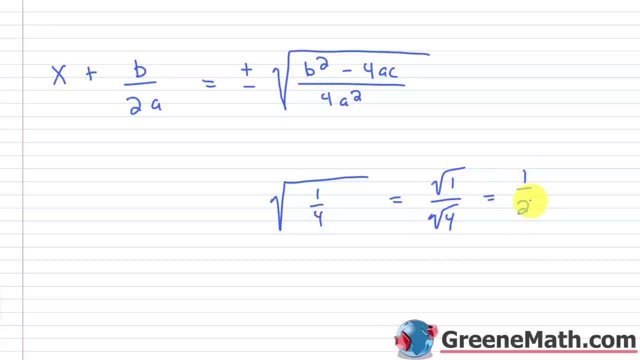 which is equal to 1 over 2 or 1 half. So I can do the same thing here, So I can write this as plus or minus. that can stay just with the numerator, the square root of b squared minus 4ac. 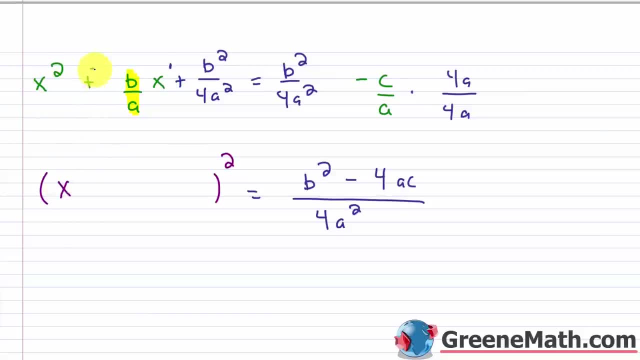 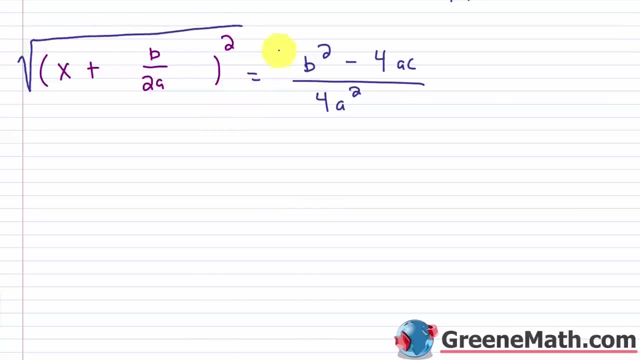 factor this guy. We know the first position would be x, and then there's a plus there, and then a minus. So we're going to factor this guy, and then there's a plus there, and then a minus. So we're going to factor this guy, and then there's a plus there, in this position the square root of b squared is b the square root of 4a squared is 2a so now what I want to do is use my square root property let me take the square root of this side and I'm going to go plus or minus the square root of this side and of course this is going to cancel with this 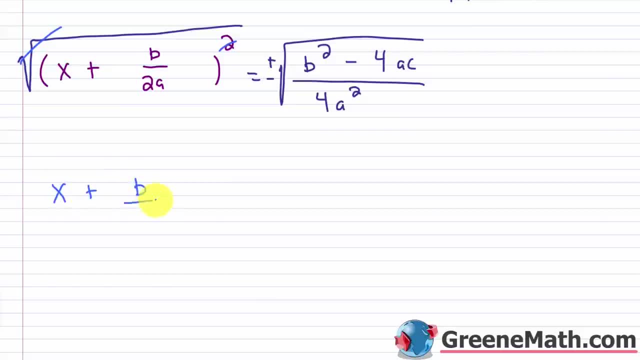 and I'm going to have x plus b over 2a is equal to plus or minus the square root of 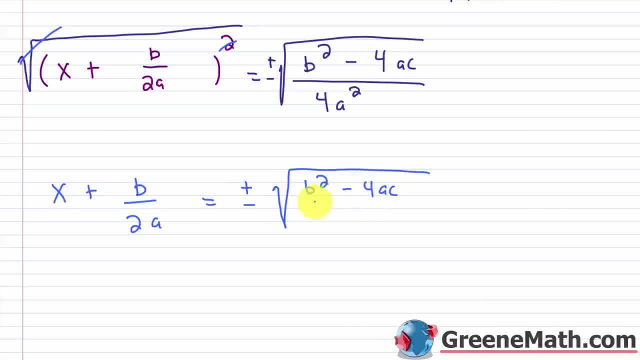 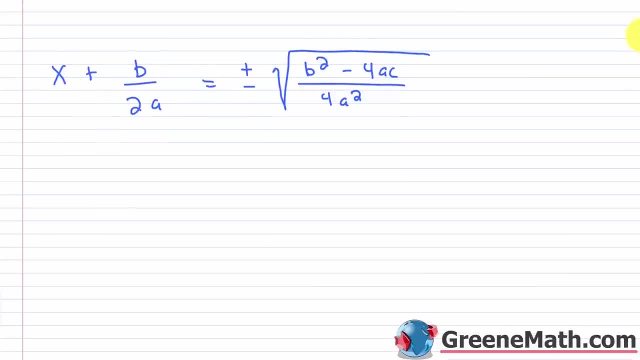 b squared minus 4ac over 4a squared all right let's scroll down and one of the things we can 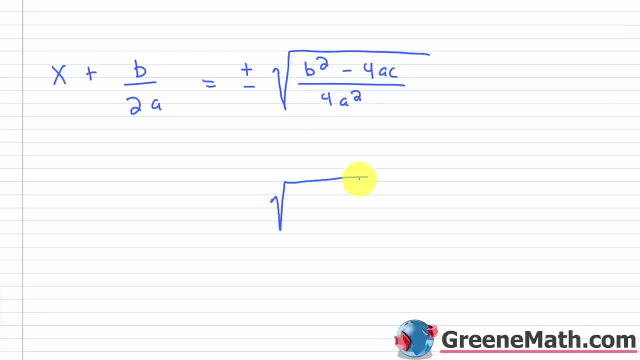 do is we can break this up right I know if I have the square root of let's say 1 4th this is equal to the square root of 1 over the square root of 4 which is equal to 1 over 2 or 1 half so I can do the same thing here so I can write this as plus 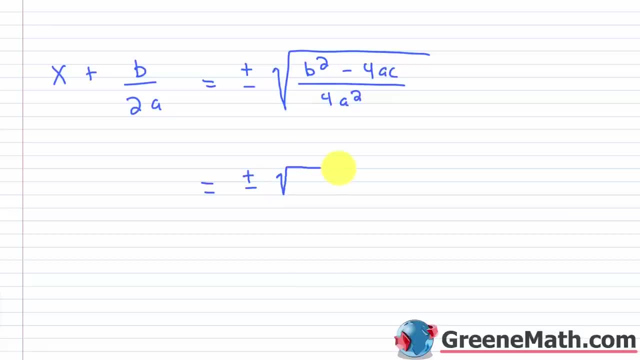 plus or minus that can stay just with the numerator the square root of b squared minus 4ac over the square root of 4a squared and over here on the left this isn't going to change we just have x plus b over 2a now why did I say this can just stay in the numerator well just assume for 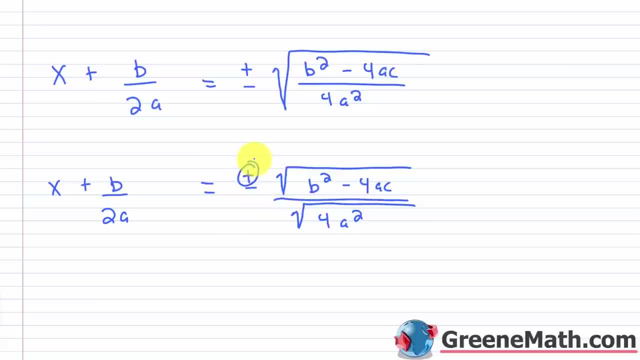 a minute that everything was positive right I have the positive version well nothing would change let me just erase that real quick you just have this over this 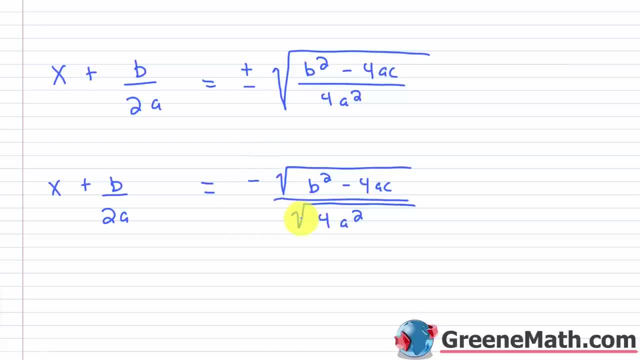 if I had the negative version well only one of them can be negative if I had a negative over a negative well then that's going to give me a positive so when you have this plus or minus it's really just out in front saying I have a positive version of this and a negative version of this so you really want one plus or minus okay so I just stick that in front of the numerator 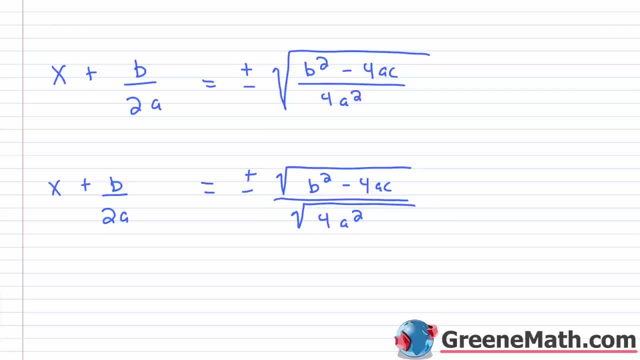 now in the denominator the square root of 4a squared would be 2a 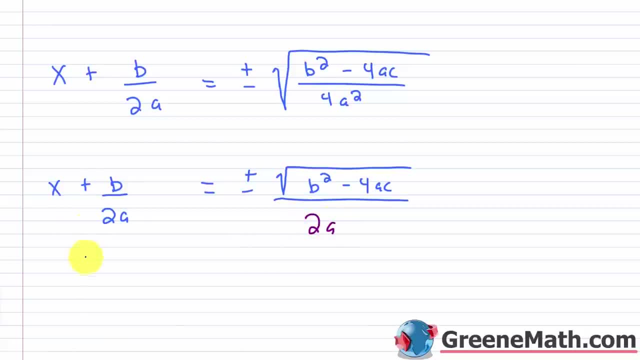 so how can I get x by itself well I can just subtract b over 2a away from each side of the 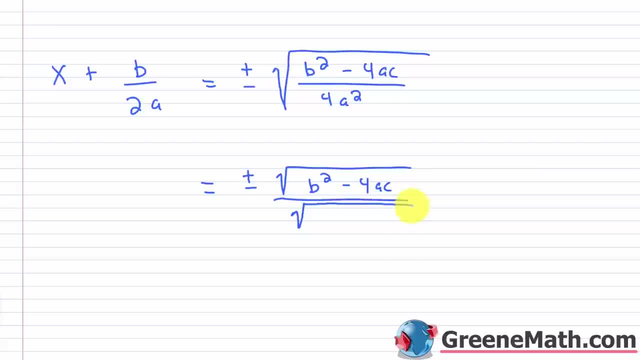 over the square root of 4a squared And over here on the left. this isn't going to change. We just have x plus b over 2a. Now why did I say this can just stay in the numerator? Well, just assume for a minute that everything was positive, right. 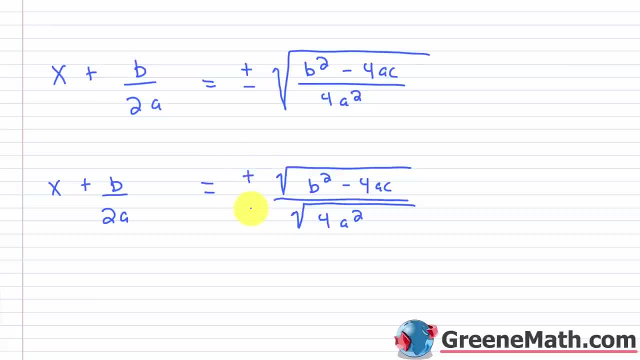 I have the positive version. Well, nothing would change. Let me just erase that real quick. You would just have this over this. I have the negative version. Well, only one of them can be negative. If I had a negative over a negative, 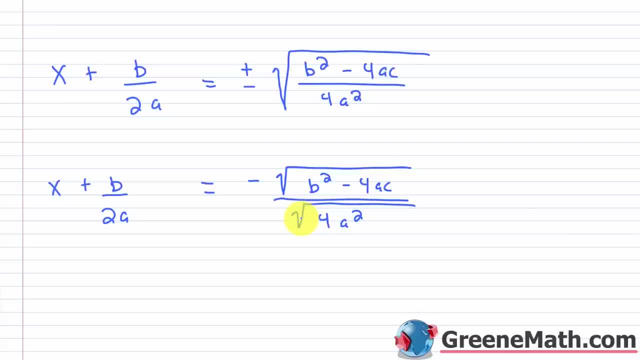 well then, that's going to give me a positive. So when you have this plus or minus, it's really just out in front saying I have a positive version of this and a negative version of this. So you really want one plus or minus. 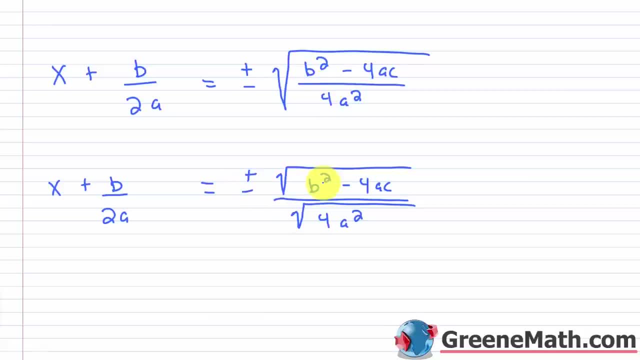 Okay, so I just stick that in front of the numerator. Now in the denominator, the square root of 4a squared would be 2a. So how can I get x by itself? Well, I can just subtract b over 2a, away from each side of the equation. 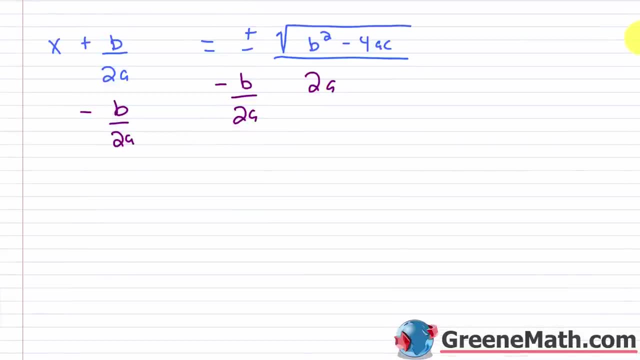 And let me scroll down a little bit. What we're going to have here this will cancel is x is equal to, I'll have negative b over 2a. Then I'll put plus, I'll have plus or minus the square root of b squared. 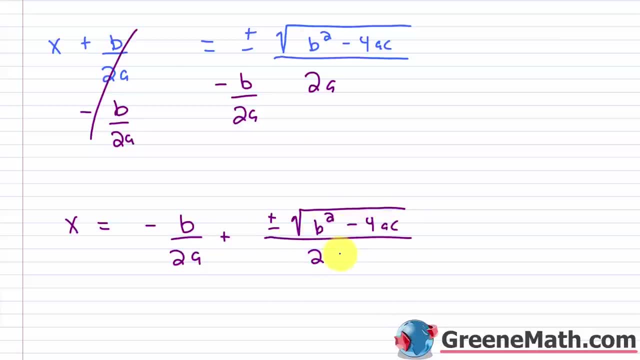 minus 2a, Minus 4ac, over 2a. Now I have a common denominator here. I have 2a here and 2a here, So really I can write this in a more compact form And in the format you're going to see in your textbook. 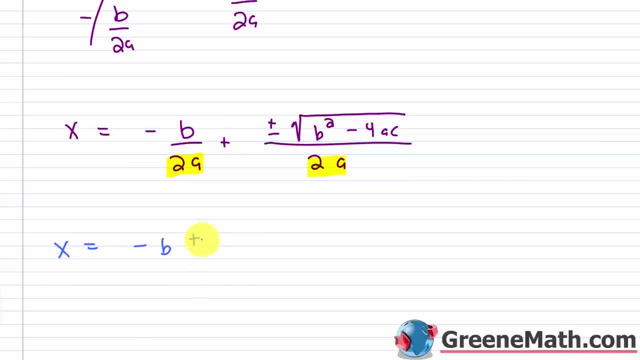 as x is equal to negative b plus or minus, the square root of b squared minus 4ac over the common denominator of 2a, And you might say: well, you don't have to do that. Yeah, you solved it for x. but what is this? 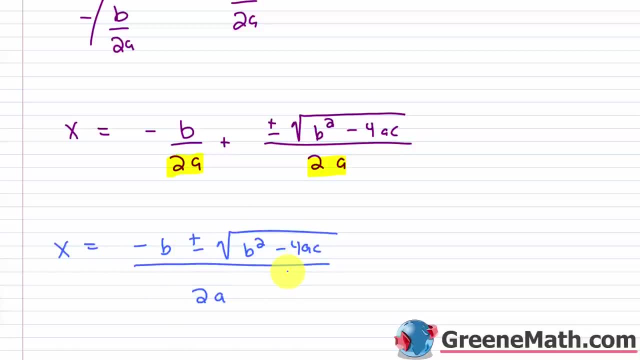 This looks like a bunch of nonsense. All I need to do to get the solution for a quadratic equation is plug in. So you remember when we saw the quadratic equation in standard form that a, b and c represented real numbers. It's just a restriction where a cannot be 0. 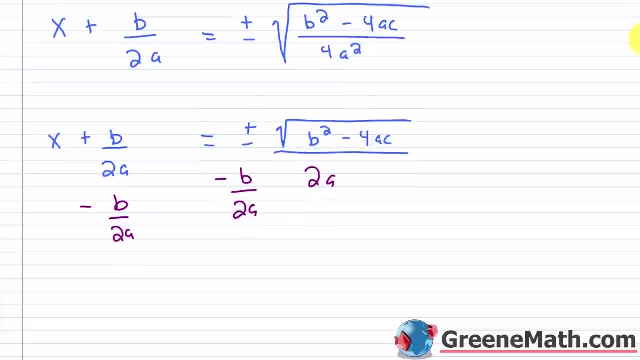 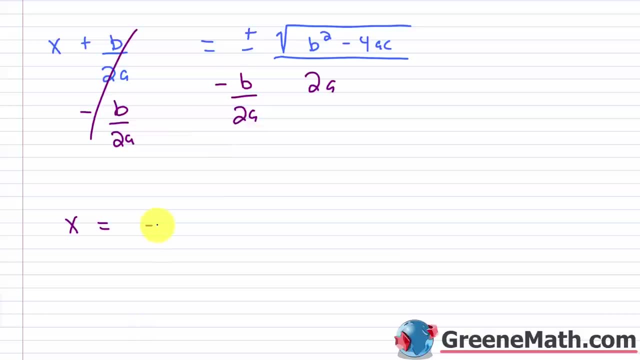 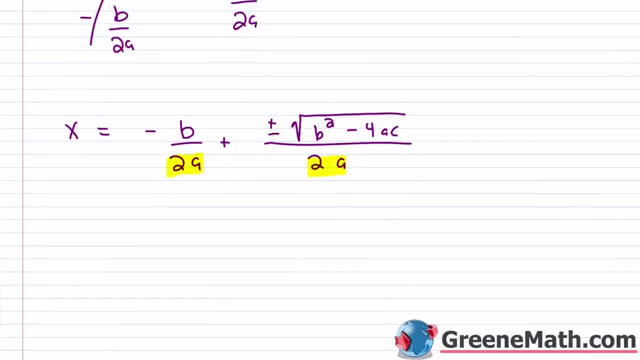 equation and let me scroll down a little bit what we're going to have here this will cancel is x is equal to I'll have negative b over 2a then I'll put plus I'll have plus or minus the square root of b squared minus 4ac over 2a now I have a common denominator here I have 2a here and 2a here so really I can write this in a more compact form and in the format you're going to see in your textbook as x is equal to negative b plus or minus the square root of b squared minus 4ac over the common denominator 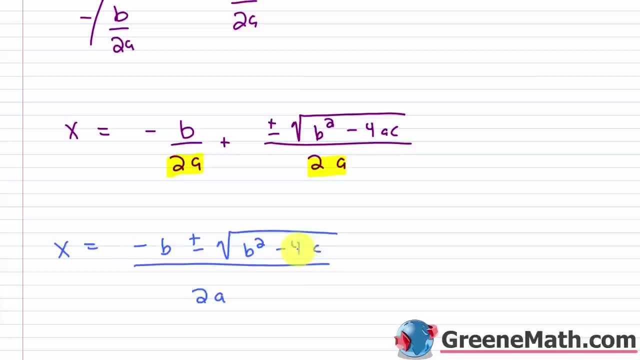 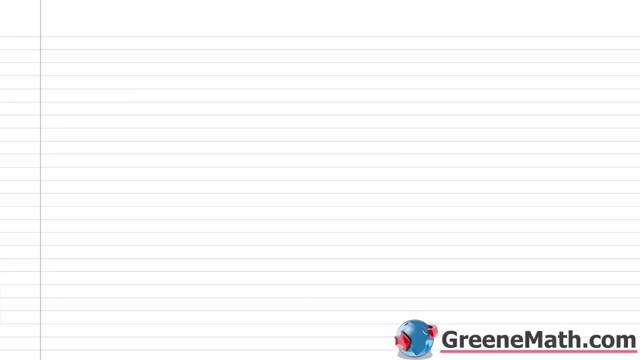 of 2a and you might say well yeah you solved it for x but what is this this looks like a bunch of nonsense all I need to do to get the solution for a quadratic equation is plug in so you remember when we saw the quadratic equation in standard form that a b and c represented real numbers right it's just a restriction where a cannot be 0 but if I plug in for a b and c I'm going to get a solution for my quadratic equation so let me copy this real quick and we're going to go down and I'm going to label this as the quadratic formula and let me just give you a quick example before we start kind of going into some more detail here if I saw something easy like x 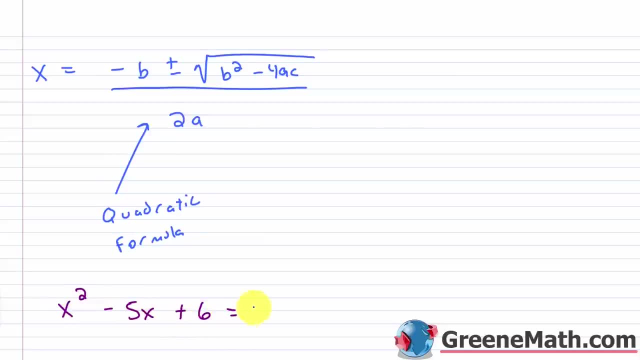 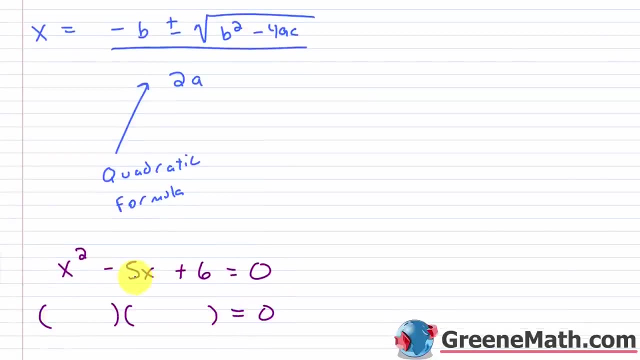 squared minus 5x plus 6 equals 0 this is something we can solve with factoring so two integers whose sum is going to be negative 5 and whose product is 6 would be negative 2 and negative 3 so we can 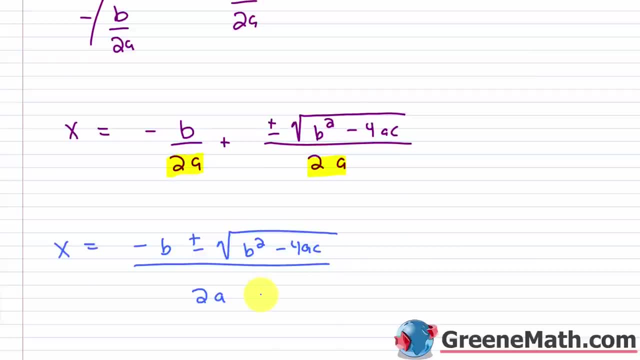 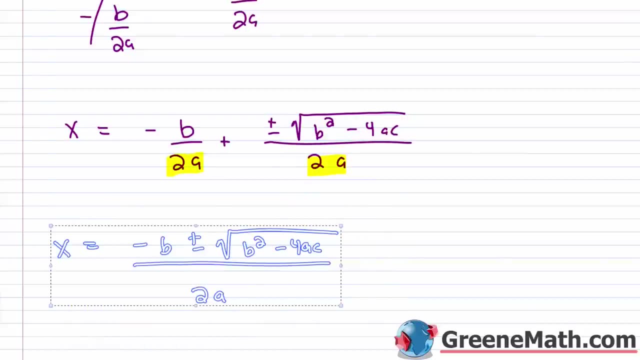 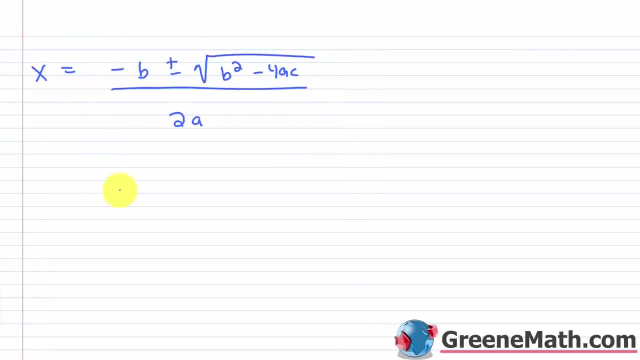 But if I plug in for a, b and c, I'm going to get a solution for my quadratic equation. So let me copy this real quick And we're going to go down And I'm going to label this as the quadratic formula. 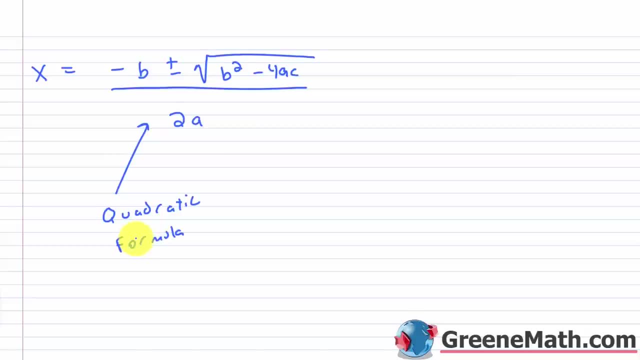 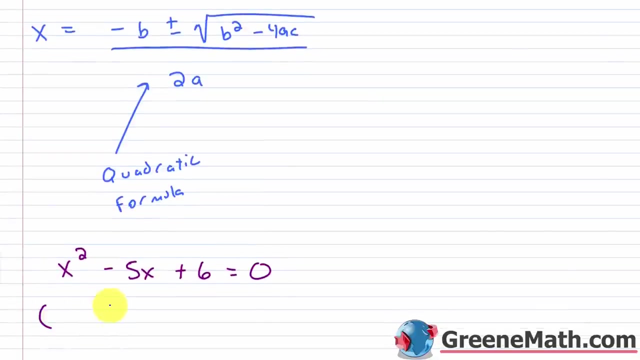 And let me just give you a quick example before we start kind of going into some more detail here. If I saw something easy like x squared minus 5x plus 6 equals 0, this is something we can solve with factoring, So two integers whose sum is going to be negative 5. 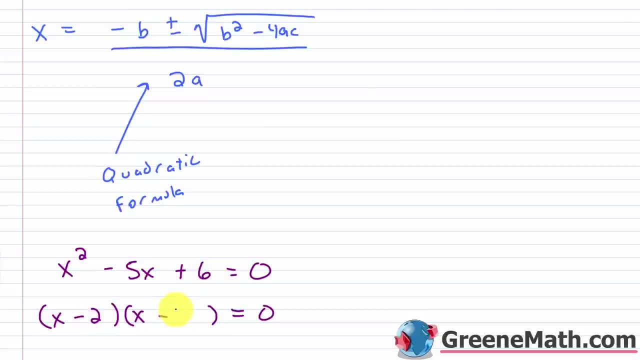 and whose product is 6, would be negative 2 and negative 3.. So we can look at this at this point and hopefully know that the solutions would be x equals 2 or x equals 3.. And that's at each one of these equal to 0.. 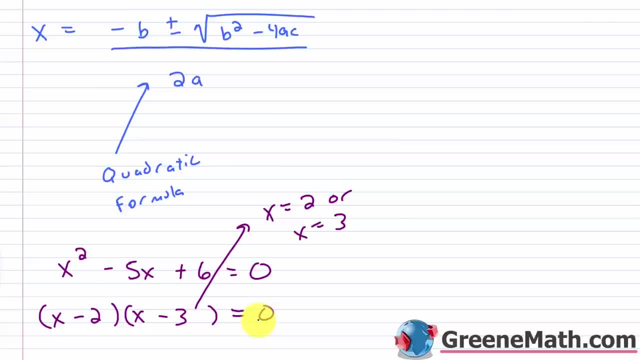 And I'd solve If I plugged into the quadratic formula. all I would need to do is say okay. a generic quadratic equation of standard form is: ax squared plus bx plus c equals 0. So in this case, in this case, a is equal to what? 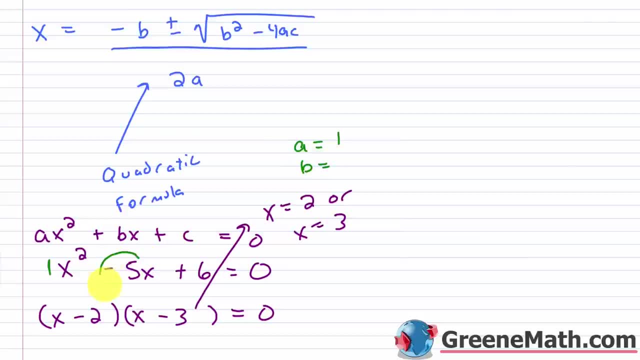 It's equal to 1.. b is equal to what It's equal to negative 5.. And c is equal to what It's equal to 6.. All right, I'm just lining things up with that generic example. So now I would just plug into the formula. 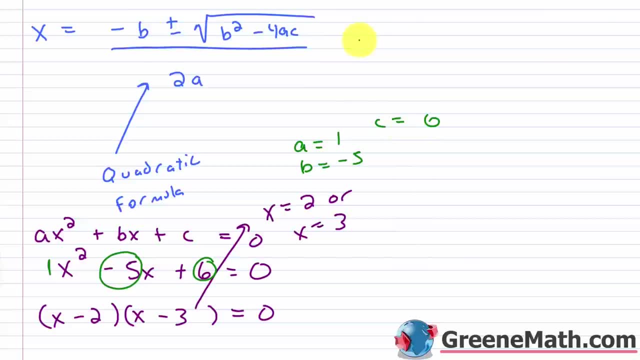 So I would have: x is equal to Negative b. The negative of negative 5 is positive 5.. So I'd have negative, negative 5.. Again, that's positive 5.. Then you have plus or minus. So I'm going to do the positive scenario first. 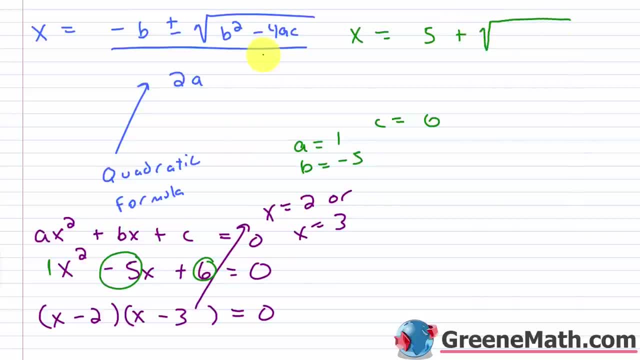 So, plus the square root of You have b squared, Negative 5 squared is 25.. Minus 4 times a, times c, 4 times 1 is 4.. Times 6 is 24.. Then this is all over. 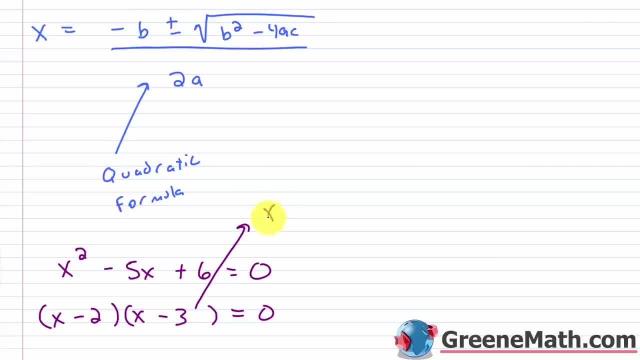 look at this at this point and hopefully know that the solutions would be x equals 2 or x equals 3 and I'd set each one of these equal to 0 and I'd solve if I plugged into the quadratic formula all I would need to do is say okay a generic quadratic equation of standard form is ax squared plus bx plus c equals 0 so in this case in this case a is equal to what it's equal to 1 b is equal to what it's equal to negative 5 and c is equal to what it's equal to 6 and I'm just lining things up with that generic example so now I would just plug into the formula so I would have x is equal to negative b the negative of negative 5 is positive so I would have x is equal to negative b so I'd have negative negative 5 again that's positive 5 then you have plus or minus so I'm going to do the positive scenario first so plus the square root of you have b squared negative 5 squared is 25 minus 4 times a times c 4 times 1 is 4 times 6 is 24 then this is all over 2 times a a in this case is 1 so all over 2 so 25 minus 24 is negative 5 so I'd have negative negative 5 4 is 1 so you'd have the square root of 1 which is 1 so 5 plus 1 is 6 so you'd have 6 over 2 which equals 3 which is one of your solutions right there now if we do the negative scenario the negative scenario you'd have again negative b so negative of negative 5 is 5 then minus the square root of we know this is going to be the same b squared you have negative 5 squared that's 25 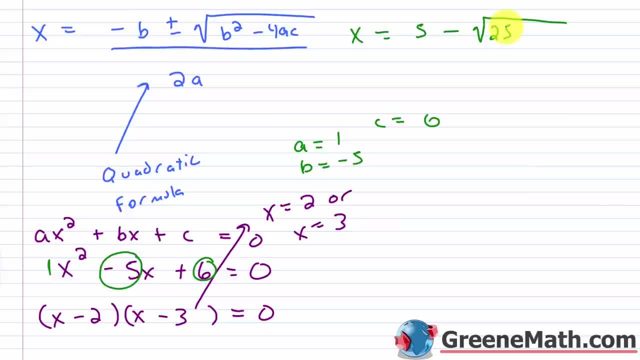 4 times a a is 1 times c c is 6 so 4 times 1 times 6 is 24 so this ends up being the square root of 1 again so this is 1 over 2 times a again a is 1 so over 2 5 minus 1 is 4 4 over 2 is 2 so that's 2 and that's how we get our other solution right there so you can see that plugging into the 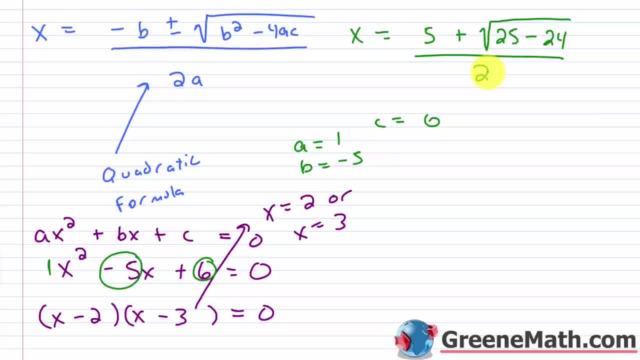 2 times a. a in this case is 1.. So all over 2.. So 25 minus 24 is 1.. So you'd have the square root of 1, which is 1.. So 5 plus 1 is 6.. 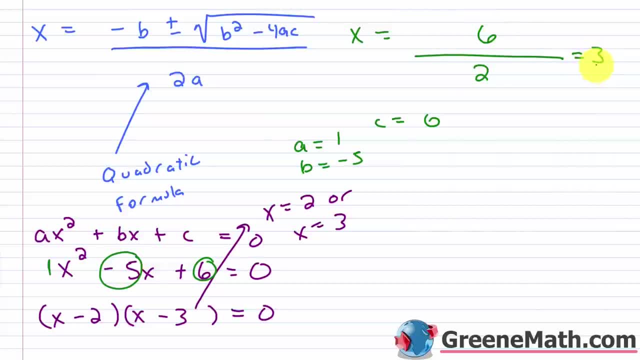 So you'd have 6 over 2,, which equals 3, which is 1 of your solutions right there. Now, if we do the negative scenario, the negative scenario, you'd have again negative b. So negative of negative 5 is 5.. 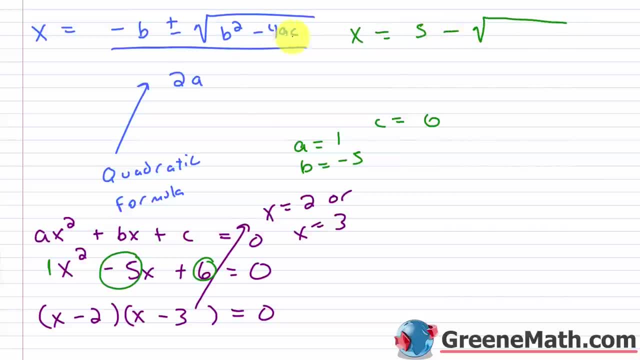 Then minus the square root of, We know this is going to be negative. This is going to be the same b squared, You have negative 5 squared, That's 25 minus 4 times a. a is 1 times c, c is 6.. 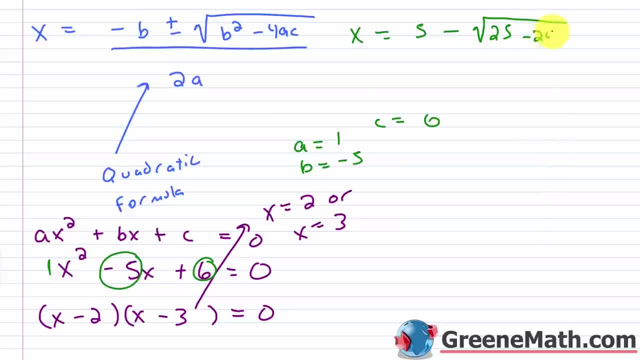 So 4 times 1 times 6 is 24.. So this ends up being the square root of 1 again. So this is 1 over 2 times a. again a is 1.. So over 2, 5 minus 1 is 4,. 4 over 2 is 2.. 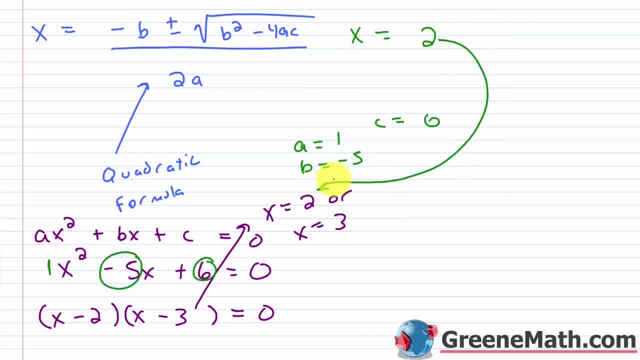 So that's 2.. And that's how we get our other solution right there. So you can see that Plugging into the quadratic formula is pretty easy. I don't need to factor anything, I don't need to complete any squares. 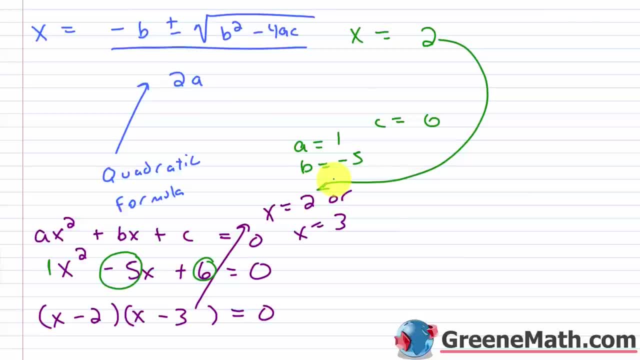 I don't need to do anything other than line up my equation in standard form, figure out what a is, b is and c is, and then plug in and get an answer. Okay, it's very, very simple. All right, so let's go through some technical details. 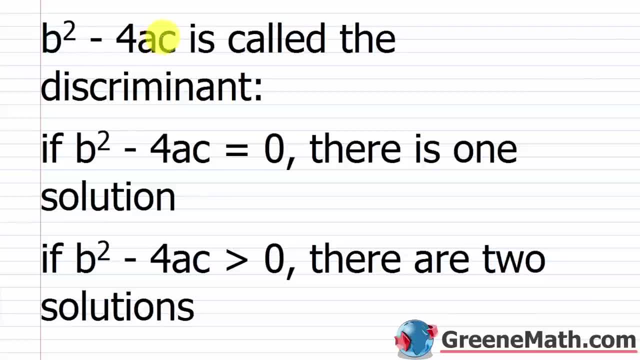 So b squared minus 4ac. this is the part that's under the square root symbol- is called the discriminant. Write that down Very, very important and it comes up a lot, especially when you get into Algebra 2 and college algebra. 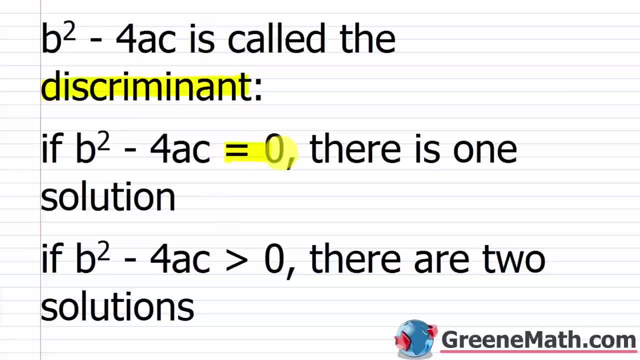 If b squared minus 4ac equals 0, there is one solution. One solution okay. If b squared minus 4ac is greater than 0,, like we just had in the last example, there are two solutions, okay, Two solutions. 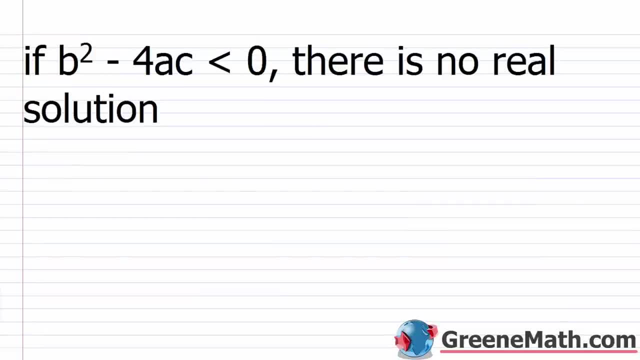 And then if b squared minus 4ac is 0,, if b squared minus 4ac is less than 0, there is no real solution. no real solution. And in some Algebra 1 courses you're going to deal with negative square roots. 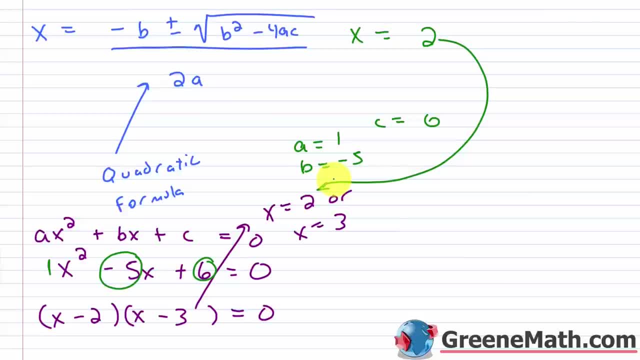 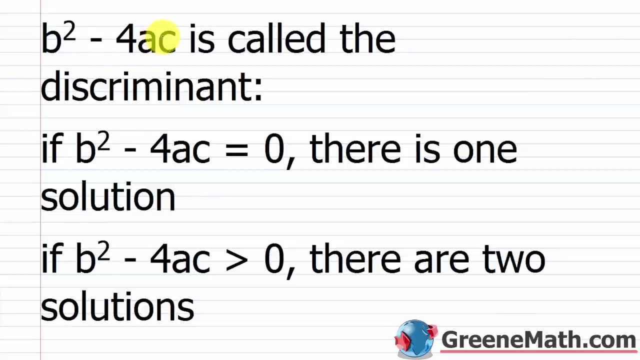 quadratic formula is pretty easy I don't need to factor anything I don't need to complete any squares I don't need to do anything other than line up my equation in standard form figure out what a is b is and c is and then plug in and get an answer okay it's very very simple all right so let's go through some technical details so b squared minus 4ac this is the part that's under the square root symbol is called the discriminant write that down very very important and it comes up a lot especially when you get into algebra 2 and college 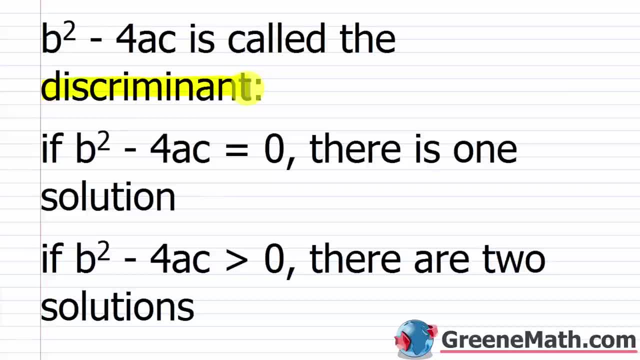 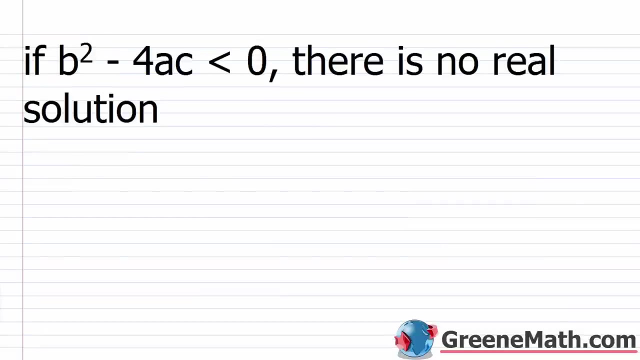 algebra if b squared minus 4ac equals 0 there is one solution one solution okay if b squared minus 4ac is greater than 0 like we just had in the last example there are two solutions a two solutions and then if b squared minus 4ac is less than 0 there is no real solution no real solution 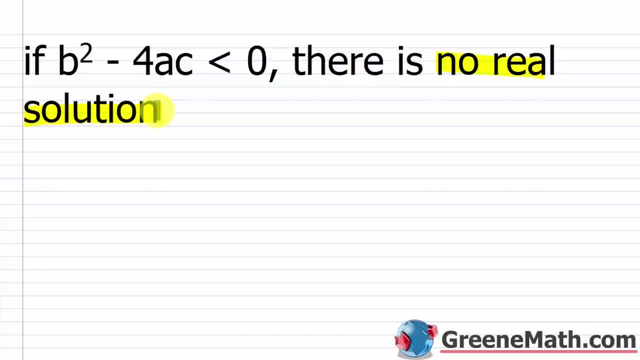 but of course we don't completely understand that so your answer going is of course not the answer we're going to have to get asked more and more in daily lectures you can all be more ask more out are nanishquits the doctor is yogurt shield 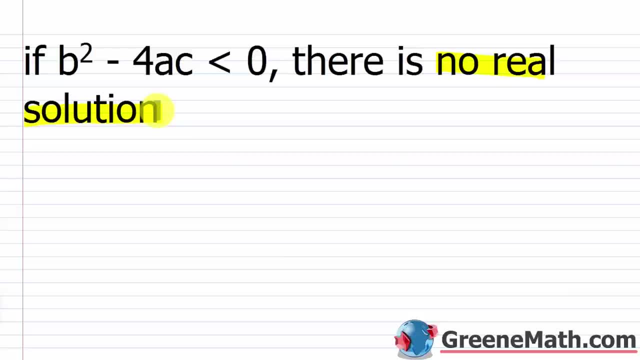 again in some algebra one courses you're going to deal with negative square roots in other algebra courses like this one I'm not gonna take it on I'm gonna wait for algebra two so that you can completely understand what's going on I've taught in algebra one before and I feel like students just don't have a good enough understanding of the basic processes to get into that so in the next course I'm going to 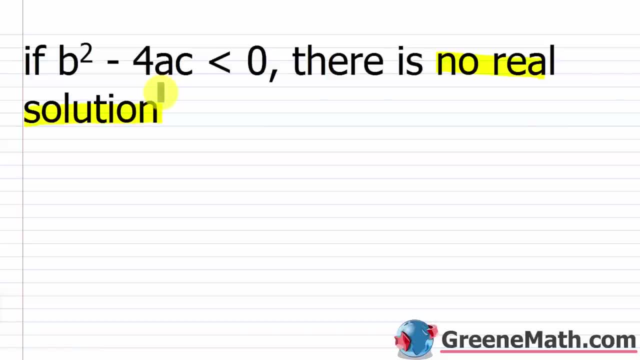 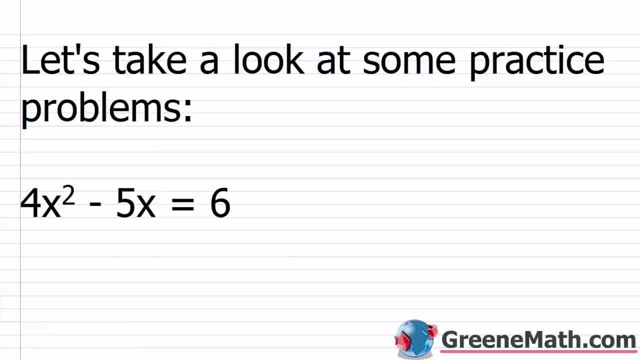 zero, there is a solution for it, but it involves the complex number system, which we just haven't covered yet. All right, so let's take a look at some practice problems. So we have 4x squared 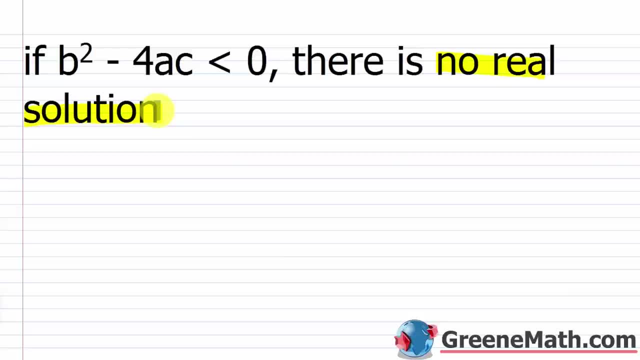 In other Algebra 1 courses like this one, I'm not going to take it on. I'm going to wait for Algebra 2 so that you can completely understand what's going on. I've taught in Algebra 1 before and I feel like students just don't have a good enough. 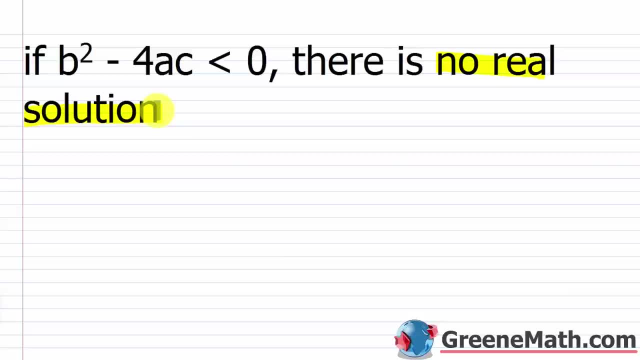 understanding of the basic processes to get into that. So in the next course I'm going to do which is going to be in the next class I'm going to do, which is Algebra 2, we are going to talk about what to do when b squared minus 4ac is less than 0.. 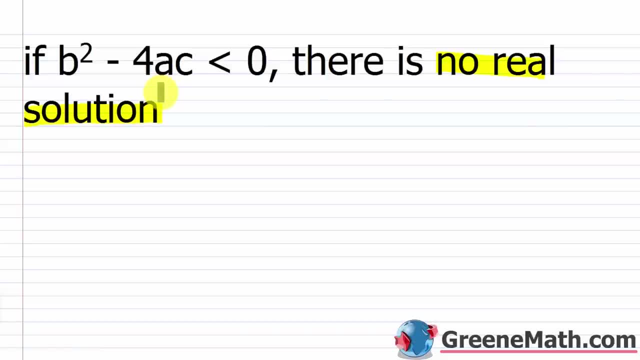 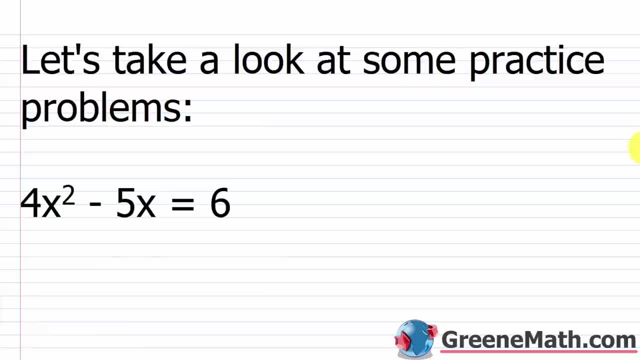 There is a solution for it, but it involves the complex number system which we just haven't covered yet. All right, so let's take a look at some practice problems. So we have 4x squared minus 5x equals 6.. 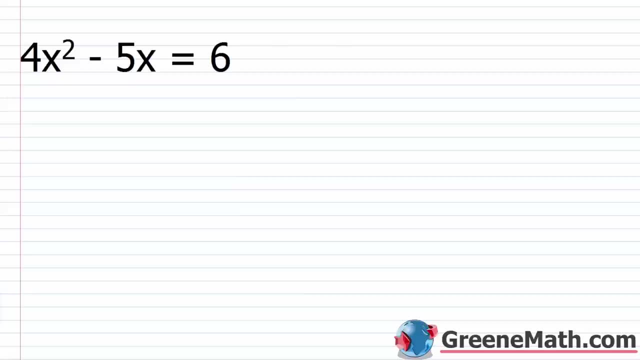 The first thing I'm going to do is I'm going to write the generic form for the quadratic equation in standard form. So I'm going to take a little flash card and it should be something that you memorize. So it's: ax squared plus bx plus c is equal to 0.. 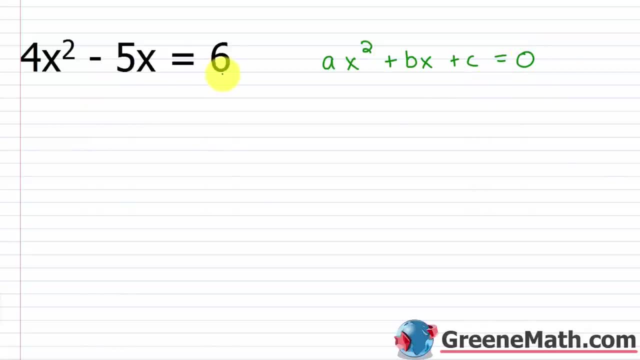 Now, this guy right here does not match this guy. okay, What we need to do is move our constant term over to the left, And again we do that. with basic algebra. We just subtract 6 away from each side of the equation. and I'm going to have- and let me just 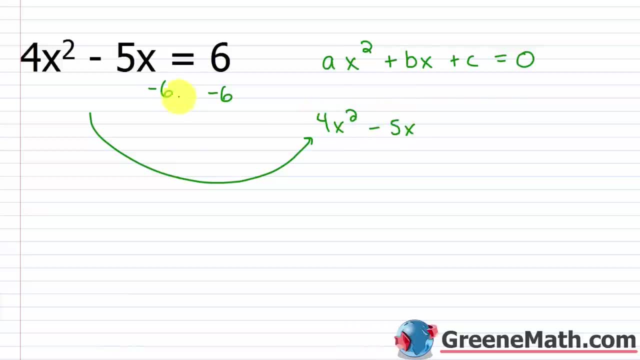 write it over here: 4x squared minus 5x Subtracted, 6 away, so minus 6.. This would cancel, so equals 0.. Now the next thing that I want to do is line everything up and I want to figure out what is a. 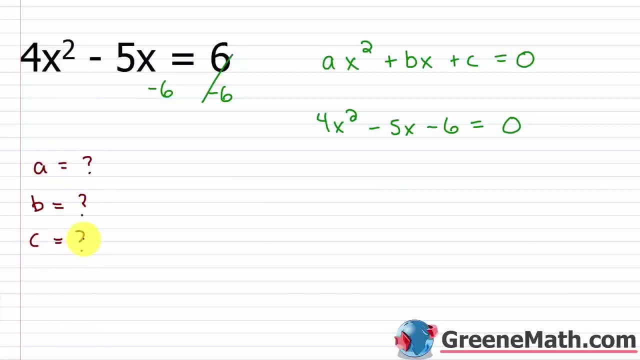 what is b and what is c? Okay, I need those to plug into the formula. So a is the coefficient for the x squared, so that's 4.. b is the coefficient for the x to the first power, so that's negative 5.. 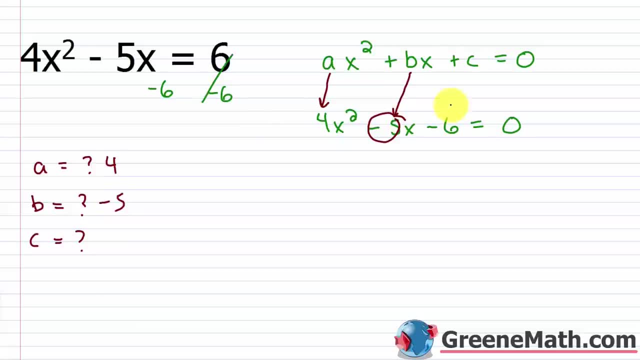 You need the negative there, Don't just put 5.. And then c is negative 6. It's the constant. You need the negative, Don't just put 6.. So once we have this information, we plug it into the quadratic formula. 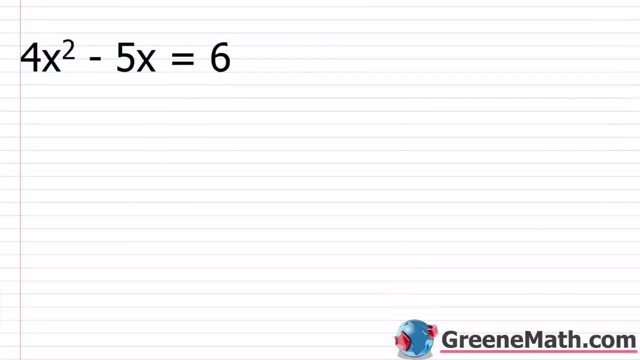 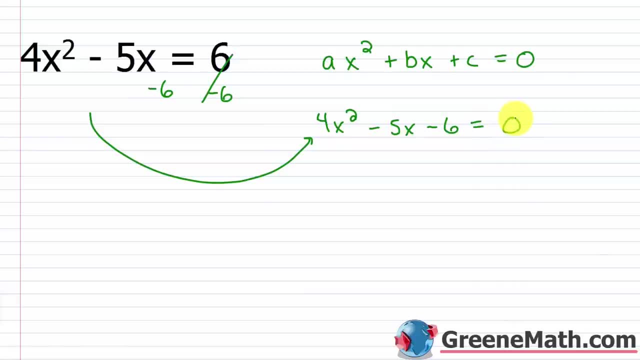 6 this would cancel so equals 0. Now the next thing that I want to do is line everything up and I want to figure out what is a what is b and what is c. Okay I need those to plug into the formula. So a is the coefficient for the x squared so that's 4. b is the coefficient for the x to the 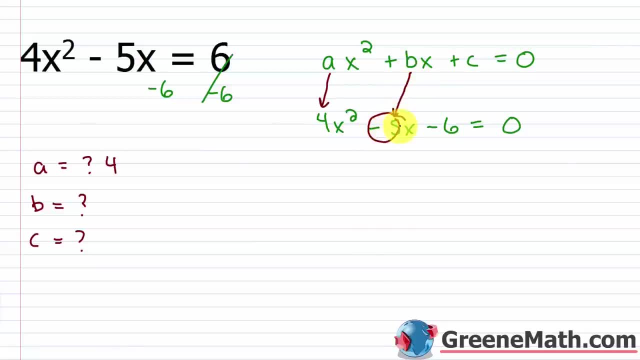 first power so that's negative 5. You need the negative there don't just put 5. And then c is negative 6. It's the constant. You need the negative don't just put 6. So once we have this 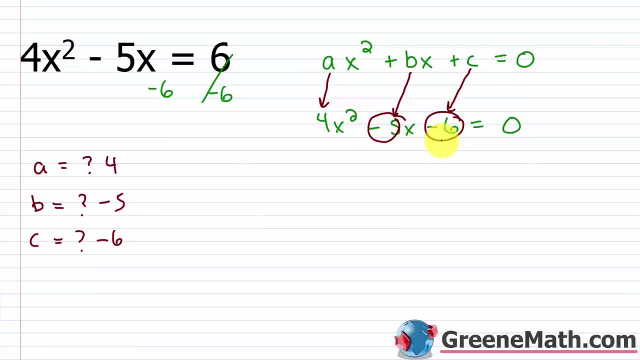 information we plug it into the quadratic formula. So again the quadratic formula is x is equal to negative b plus or minus the square root of b squared minus 4ac this is all over 2a. So what are we going to have here? We'll have x is equal to negative b. So I put negative and then for b I put negative 5 in there plus or minus the square 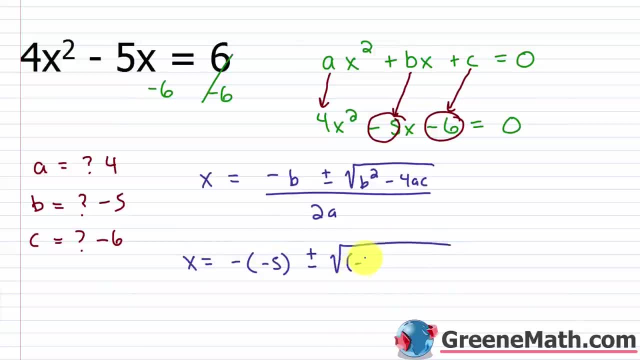 root of we have b squared. So let's put negative 5 and let's square that minus 4 times a that's 4 times c that's negative 6 and this is all over 2 times a. a is 4 so 2 times 4. 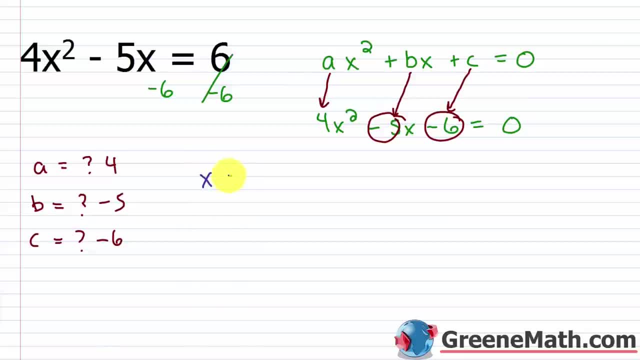 So again, the quadratic formula is: x is equal to negative b, plus or minus the square root of b. squared minus 4ac, This is all over 2a. So what are we going to have here? We'll have: x is equal to negative b. 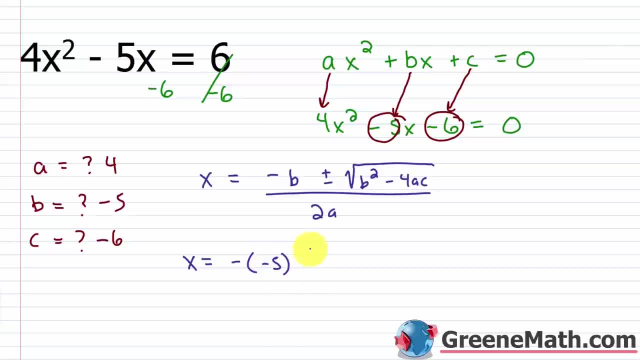 So I put negative and then for b I put negative 5. in there, Plus or minus the square root of we have b squared. So let's put negative 5, and let's square that Minus 4 times a, that's 4.. 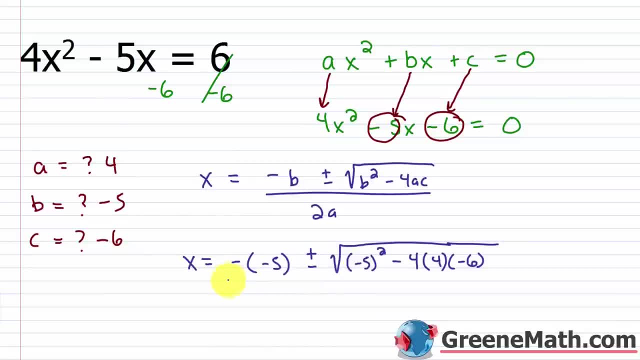 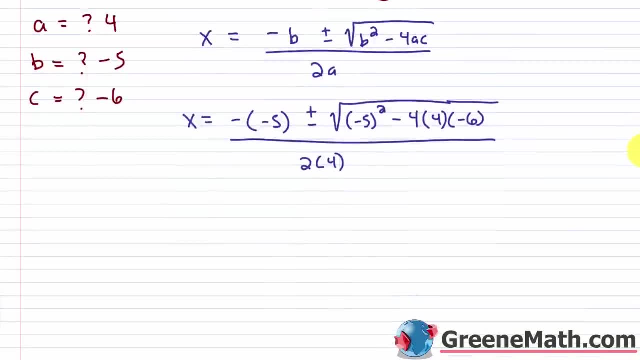 Times c, that's negative 6.. And this is all over 2 times a. a is 4, so 2 times 4.. All right, so this is the first scenario. So then x is equal to the negative of negative. 5 is 5, plus the square root of negative 5. 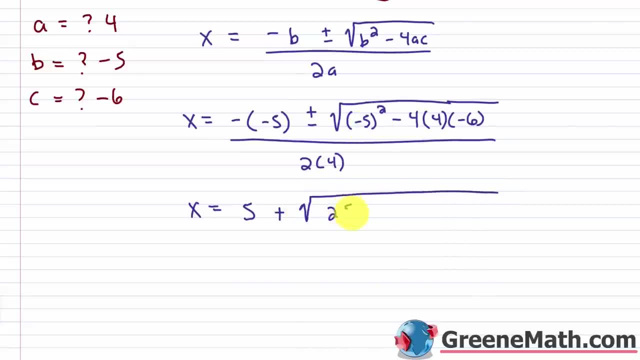 squared is 25 minus 4 times 4 is 16.. 16 times negative 6 is negative 96. So you'd have minus negative 96, or plus 96. So if I add these two together I'm going to get 121, then this is over. 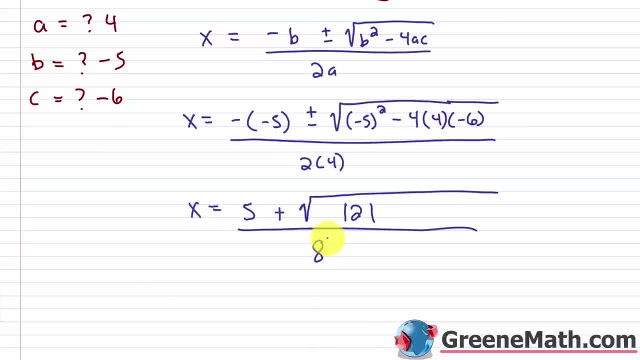 2 times 4 is 8.. Now, what we just talked about was that negative 5 is 5, and this is 4 times, 3 times that. You don't have to do the final question, You just have to solve the games at the end. OK, All right, So that's pretty much it. Take a look at the satisfying explanation. All right, we're going to go accept these 2 equations at the bottom. Let's do it right away. Okay, So we're going to take these over. as we know, the expression. 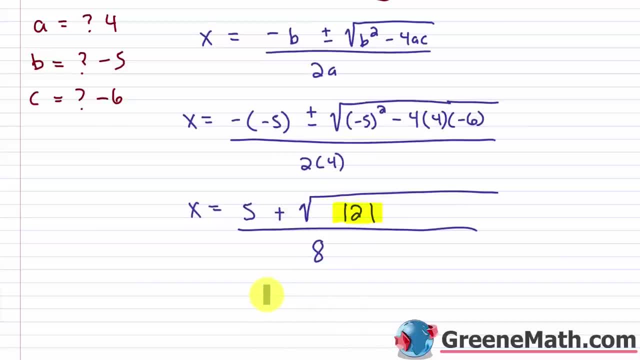 OK was that. if the result of this in here is greater than zero, I'm gonna have two solutions. if it equals zero, I have one solution. why is that the case? because the square root of zero would be zero. this would be gone, and I just have in. 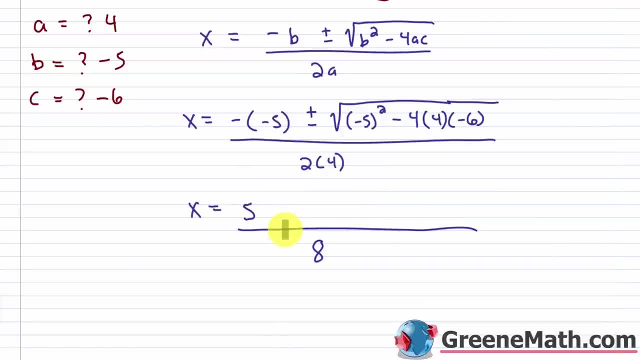 this case. if that did happen, I'd have 5 over 8. okay, that's not the case here. I have the square root of 121, which is 11, so this is 11. 5 plus 11 is 16: 16 over 8. 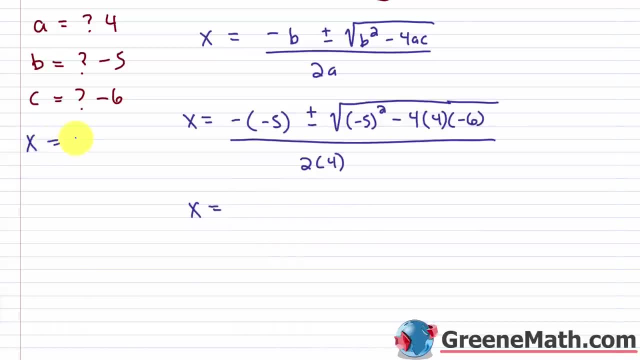 is 2, so I get X equals 2 as one of my solutions. then for the other solution, this would all be the same. so negative of negative 5 is 5, I'd use minus now. so minus the square root of we know this turns out to be 121, so let's just put. 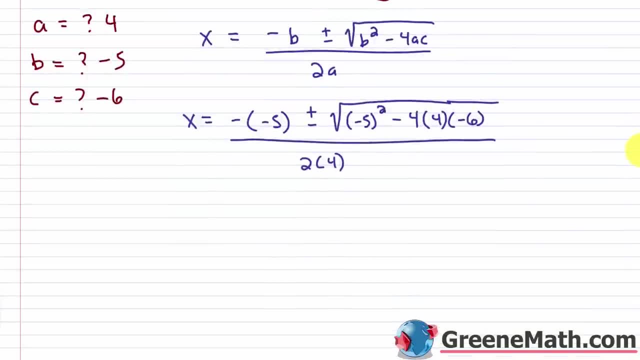 Alright so this is the first scenario. So then x is equal to the negative of negative 5 is 5 plus the square root of negative 5 squared is 25 minus 4 times 4 is 16. 16 times negative 6 is negative 96. So you'd have minus negative 96 or plus 96. So if I add these two together I'm going to get 121. Then this is over 2 times 4 is 8. Now what we just talked about was that if the result of this in here is greater than 0 I'm going to have two solutions. If it equals 0 I have one solution. Why is that the case? Because the square root of 0 would be 0. This would be gone and I'd just have in this case if that did happen I'd have 5 over 8. Okay that's not the case here. I have the square root of 121 which is 11. So this is 11. 5 plus 11 is 16. 16 over 8 is 16. So this is 8 over 8 is 2. So I get x equals 2 as one of my solutions. Then for the other solution this would all be the same. So negative of negative 5 is 5. I'd use minus now. So minus the square root of. We know this turns out to be 121 so let's just put minus 11 over 8. So 5 minus 11 is negative 6. So this would be negative 6 over 8 which would reduce to negative 3 fourths. 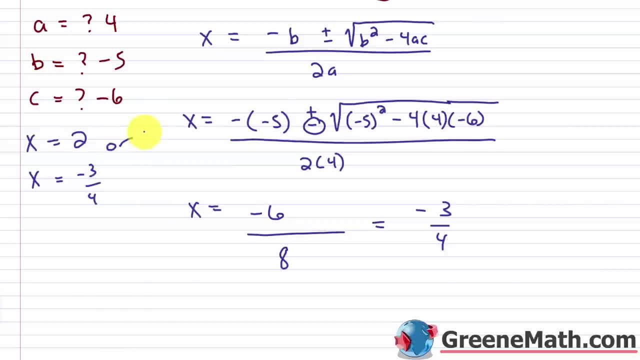 So we get x equals negative 3 fourths. Okay so pretty easy overall. Let me erase all this. With these they're pretty tedious to check. So I'm not going to check all of them but 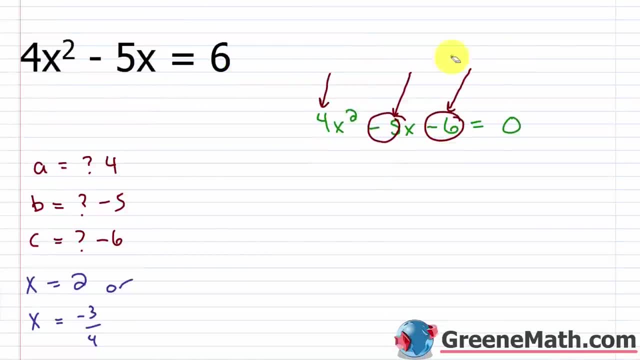 I am going to check one of them. So let's go ahead and check this one. So we know how to check things at this point. We take our answer which in this case is 2 for x and we plug it in. So plug a 2 in there and there. We'll make sure the left and the right side are equal. 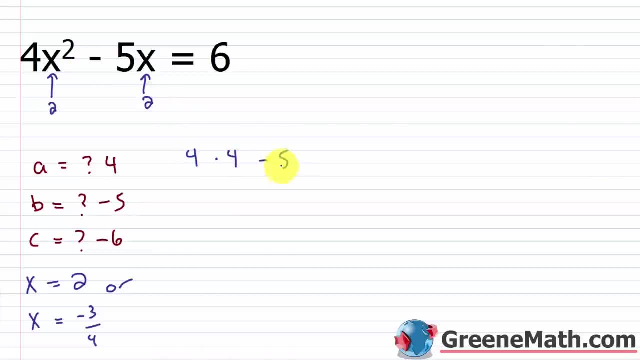 So the answer is 5 over 4 times 2 squared would be 4 minus 5 times 2 should be equal to 6. 4 times 4 is 16. 5 times 2 is 10. 16 minus 10 is 6. So you get 6 equals 6. So this solution does check out. 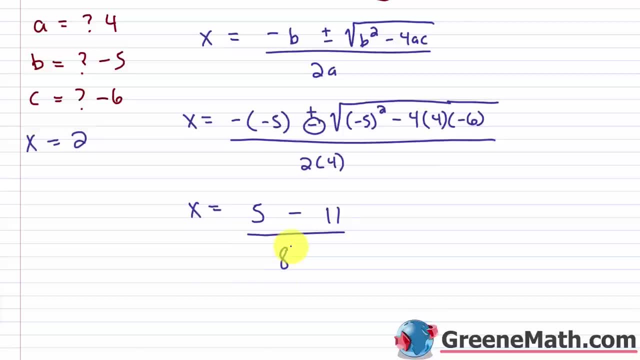 minus 11 over 8. so 5 minus 11 is negative 6. so this would be negative 6 over 8, which would reduce to negative 3 fourths you. so we get X equals negative 3 points. okay, so pretty easy overall. let me erase. 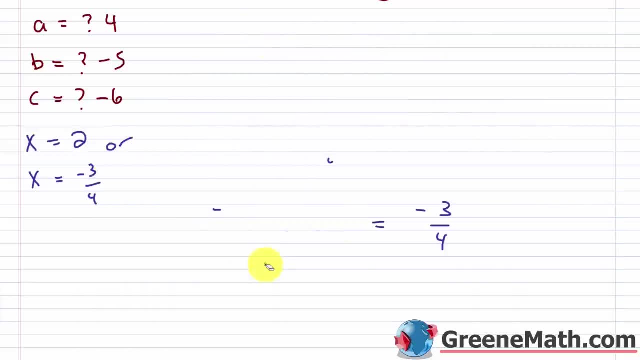 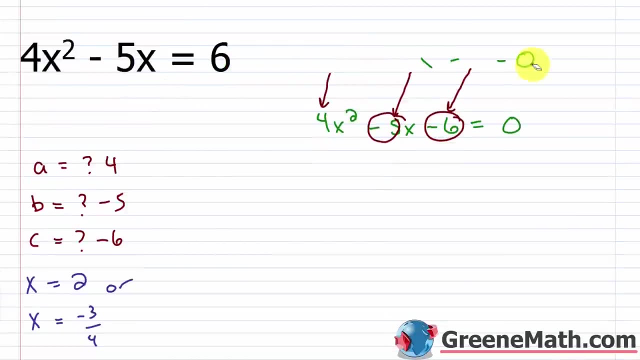 all this with these. they're pretty tedious to check, so I'm not gonna check all of them, but I am gonna check one of them. so let's go ahead and check this one, so we know how to check things. at this point we take our answer, which in: 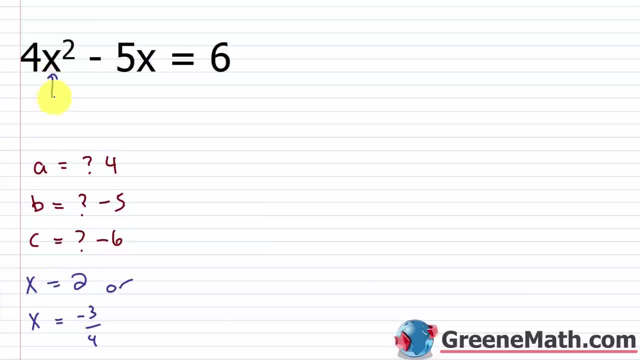 this case is 2 for X and we plug it in. so plug a 2 in there and there we'll make sure the left on the right side are equal. so X equals 9 times 6, and let me just check this one. be great. so ahead and test. 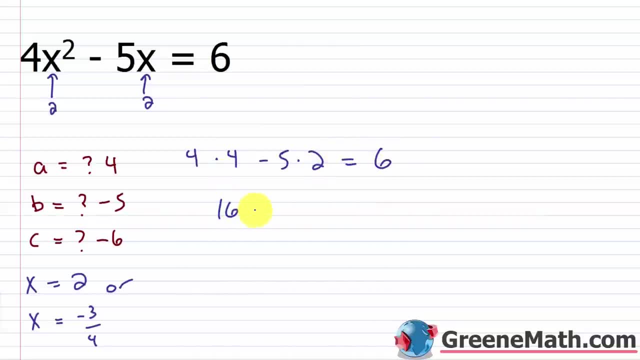 uth. so okay, right, so let's type this one in. oh my god, this is times of x minus 4. so right now, let's have some other hope if friends of mine that aren't registered in eighth grade. this is what we're doing, so we're going to take our 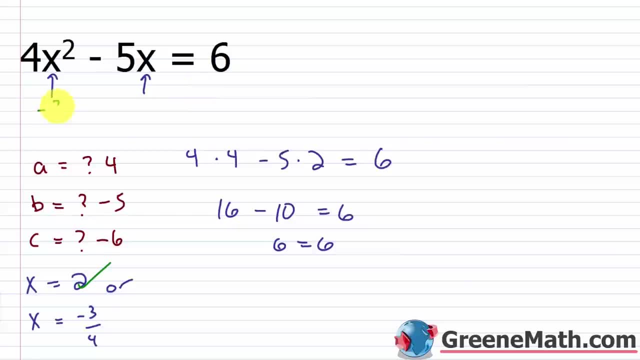 answer f forин. this one is positive 4 plus negative 4. we know this is our first answer. so x plus negative 4, so y plus minus 2. we know this is our first answer, so notify the librarian who wants answers. let's say it's positive four. 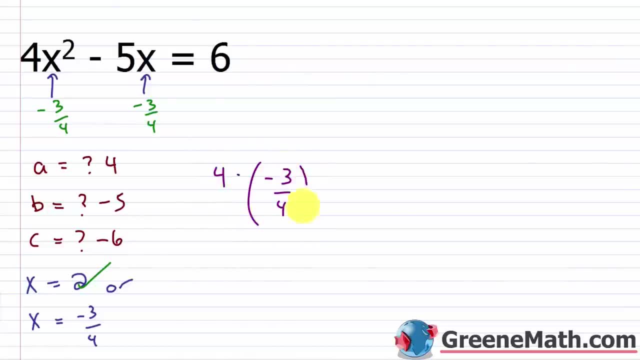 times, you'd have negative three fourths, and this is squared. and then minus five times negative three fourths and this equals six. so if i squared this guy, i'd have nine sixteenths. so times nine sixteenths and of course this would cancel with this and give me a four, so i'd have nine fourths. 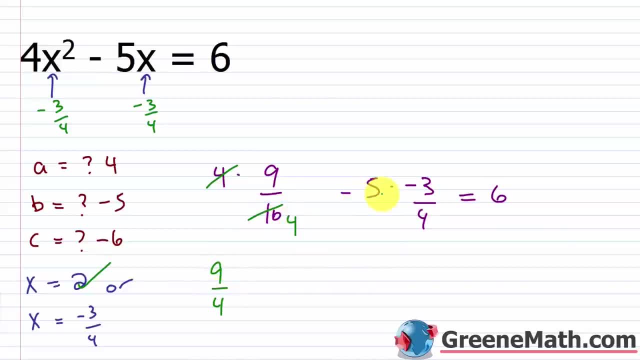 there you have basically negative five times negative, three fourths negative five times three is positive. 15 over four equals six. nine plus 15 is 24. you'd have 24 over four, which is six. again you get six equals six. so this checks out as well. so x here is equal to two or x is. 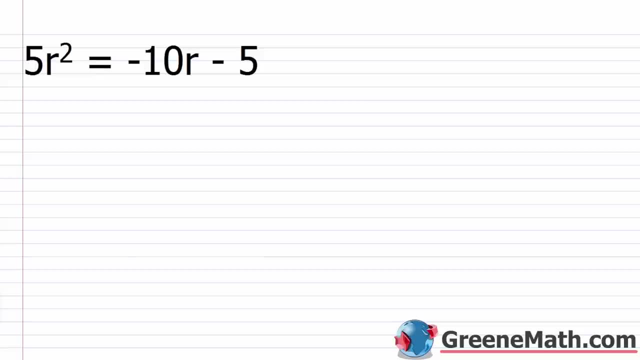 equal to negative three fourths. okay, let's go ahead and take a look at the next example. so we have five r squared is equal to negative 10r minus five. so the main thing here is that You don't want to get confused, because the variable is not an x. 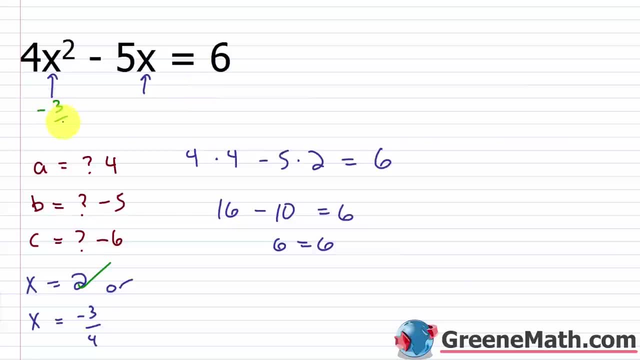 Then the other one is negative 3 fourths. So let's erase this. And so we have 4 times. You'd have negative 3 fourths. three fourths and this is squared and then minus five times negative three fourths and this equals 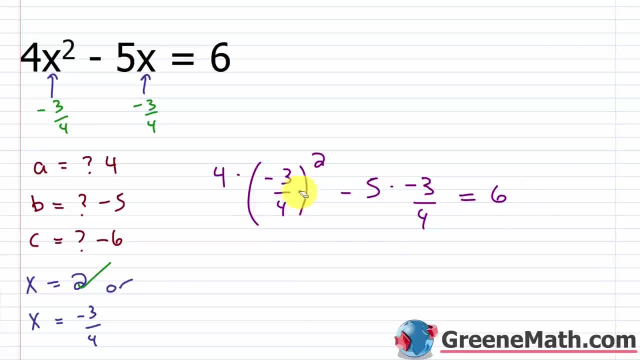 six so if i squared this guy i'd have nine sixteenths so times nine sixteenths and of course this would cancel with this and give me a four so i'd have nine fourths there you have 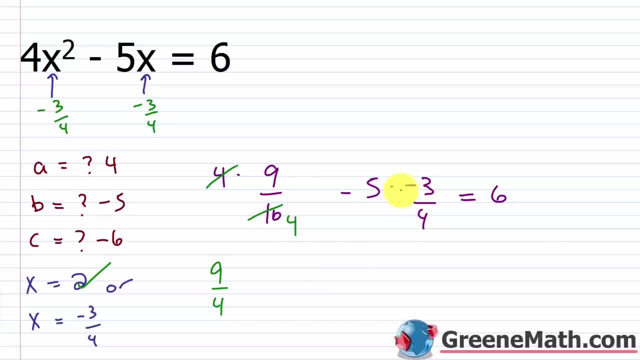 basically negative five times negative three fourths negative five times negative three is positive fifteen over four equals six nine plus fifteen is twenty four you'd have twenty four 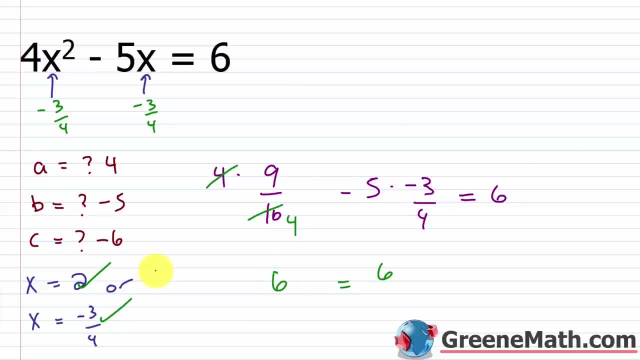 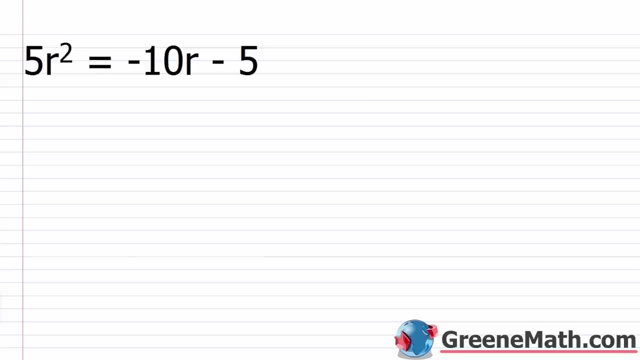 over four which is six again you get six equals six so this checks out as well so x here is equal to two or x is equal to negative three fourths okay let's go ahead and take a look at the next 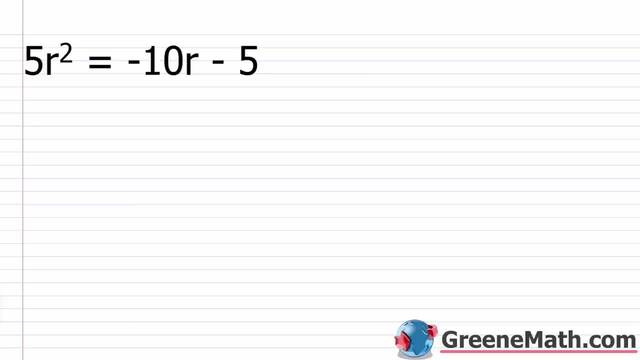 example so we have five r squared is equal to negative ten r minus five so the main thing here is that you don't want to get confused because the variable is not an x okay it doesn't matter if you have an x an r a q 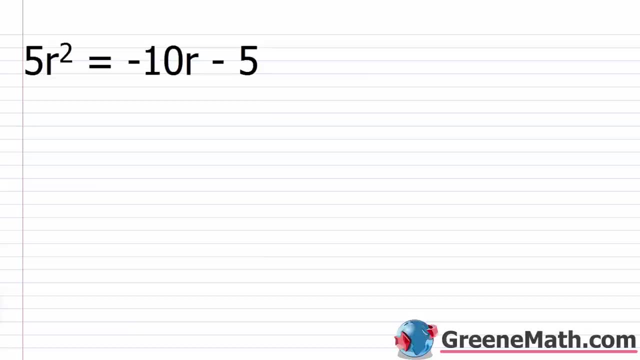 whatever it is you just follow the generic formula so if i have ax squared plus bx plus c equals zero i could rewrite this as ar squared plus br plus c equals zero it doesn't matter what the variable is we're just saying that we need to figure out what a is 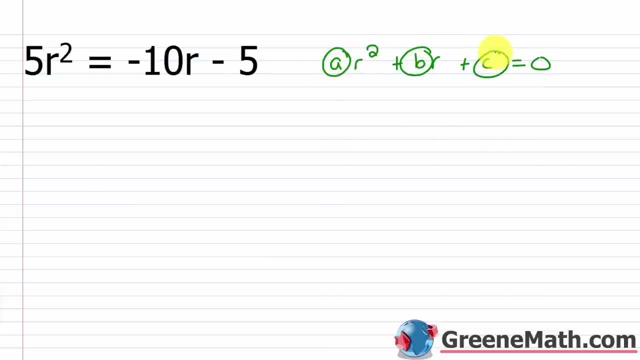 and we're going to figure out what a is and we're going to figure out what a is b is and c is so we can plug it into that formula okay so what i want to do is move these two terms over here and i'm going to do that by adding 10r to each side of the equation and i'm going to add five to each side of the equation so i would have 5r squared plus 10r plus five is equal to zero and then i can see that my a would be five this is a my b would be 10r plus 5 is equal to zero and then i can see that my a would be five this is a my b would be 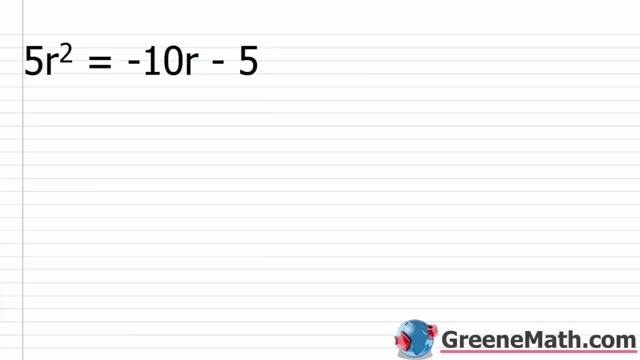 It doesn't matter if you have an x, an r, a, q, a z, whatever it is, You just follow the generic formula. So if I have ax squared plus bx plus c equals 0,. I could rewrite this as: ar squared plus br plus c equals 0.. 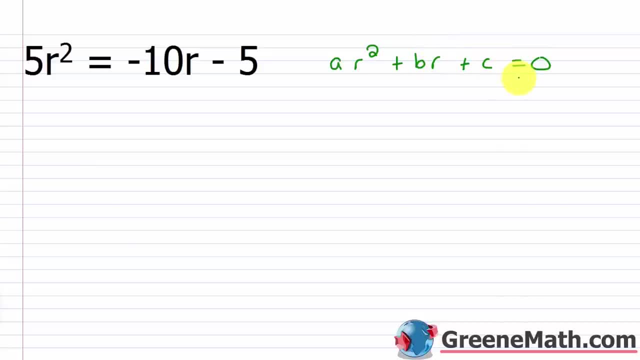 It doesn't matter what the variable is. We're just saying that we need to figure out what a is, b is and c is, so we can plug it into that formula, okay. So what I want to do is move these two terms over here. 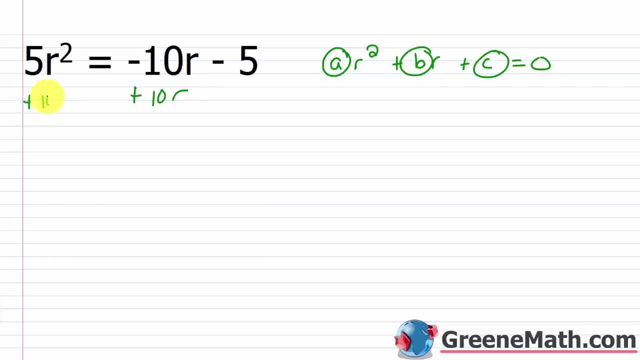 And I'm going to do that by adding 10r to each side of the equation And I'm going to add 5 to each side of the equation, So I would have 5r squared plus 10r plus 5 is equal to 0.. 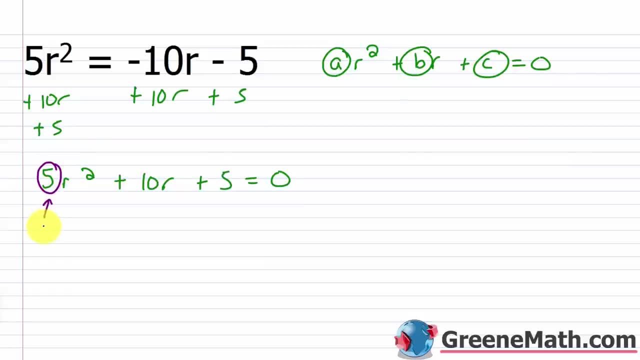 And then I can see that my x is 0.. My a would be 5.. This is a. My b would be 10.. This is b And my c would be 5.. This is c. All right, So once I know that, I can plug into the quadratic formula. 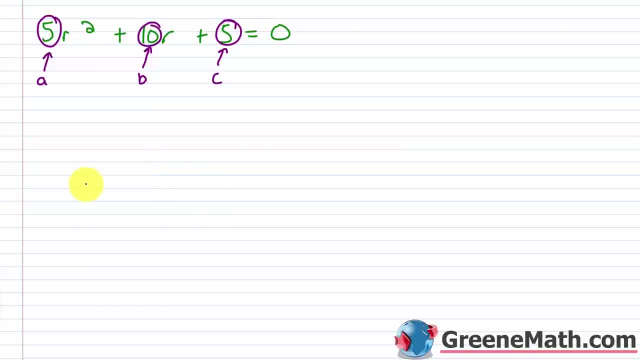 Let me scroll down And for that quadratic formula, it's usually x is equal to, but let's just say r is equal to negative b plus or minus the square root of b squared minus 4ac, This is all over 2a. 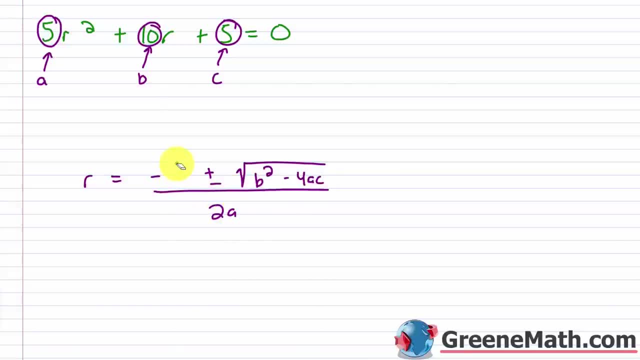 All right. So I'm going to plug in for b. So I'm going to plug in a 10 here And I'm going to plug in a 10 here. So 10 squared, let's just go ahead and put 100.. 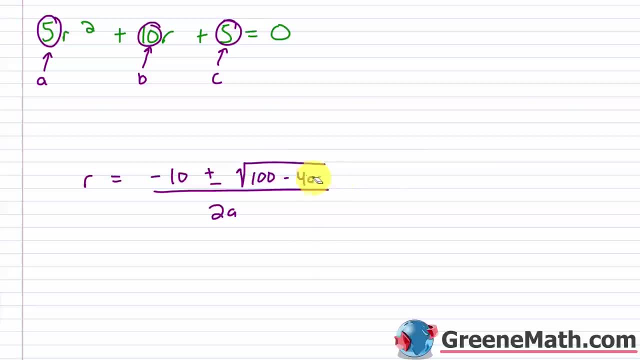 And then minus 4ac, So a is 5, c is 5.. So minus 4 times 5 times 5.. And then this is over 2a: a is 5.. So 2 times 5 is 10.. 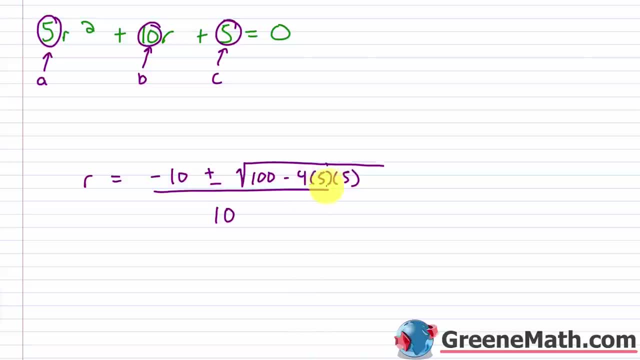 Now, the one thing you're going to notice here is that 4 times 5 is 20.. 20 times 5 is 100.. 100 minus 100 is 0.. Square root of 0 is 0.. So do I need plus or minus 0?? 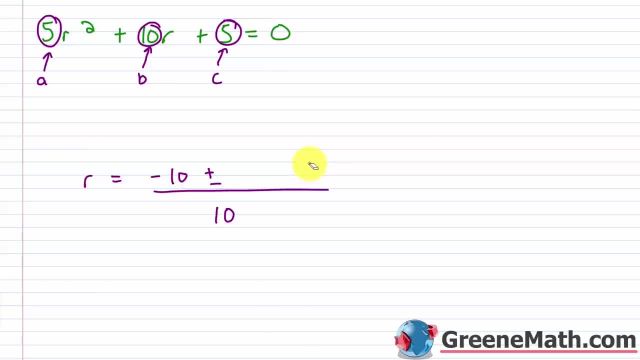 No, Because if I add 0 or I subtract 0, I'm not doing anything. It's not going to change anything. So you can erase this, And I told you that a minute ago. If b squared minus 4ac, if the discriminant, as it's called, is equal to 0, you're going to have only one solution. 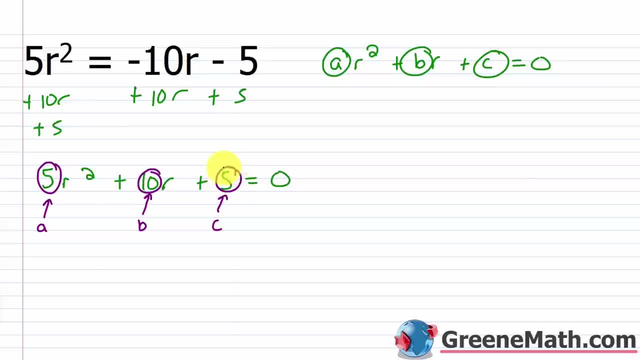 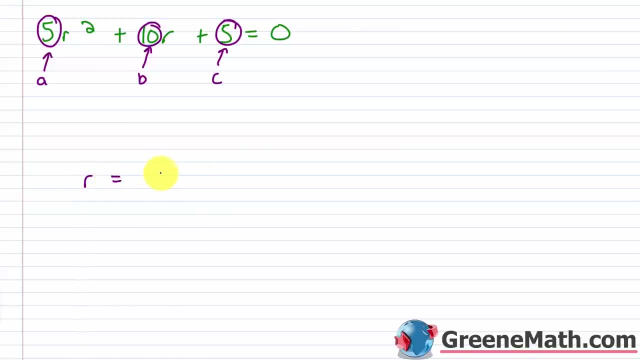 10, this is b, and my c would be 5, this is c. Alright, so once I know that, I can plug into the quadratic formula. Let me scroll down, and for that quadratic formula, it's usually x is equal to, but let's just say r is equal to negative b plus or minus the square root of b squared minus 4ac, and this is all over 2a. Alright, so I'm going to plug in for b, so I'm going to plug in a 10 here, and I'm going to plug in a 10 here, so 10 squared, let's just go ahead and put 100, and then minus 4ac, so a is 5, c is 5, so minus 4 times 5 times 5, and then this is over 2a, a is 5, so 2 times 5 is 10. Now 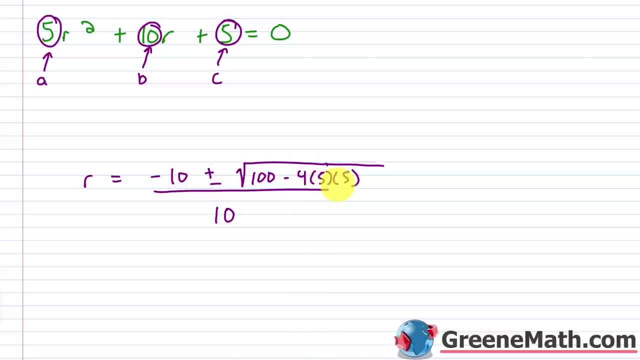 the one thing you're going to notice here is that 4 times 5 is 20, 20 times 5 is 100, 100 minus 100 is 0, square root of 0 is 0. 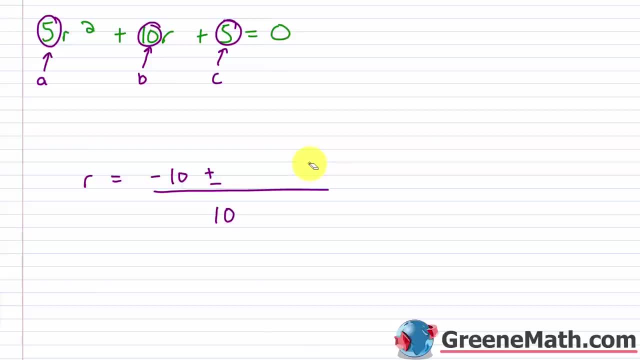 So do I need plus or minus 0? No, because if I add 0 or I subtract 0, I'm not doing anything, right? It's not going to change anything, so you can erase this, and I told you that a minute ago. If b squared minus 4ac, if the discriminant, as it's called, is equal to 0, you're going to have only one solution. So here, r is equal to negative 10 over 10, which is negative 1. And that's a simple one to check, so let's go ahead and do that. 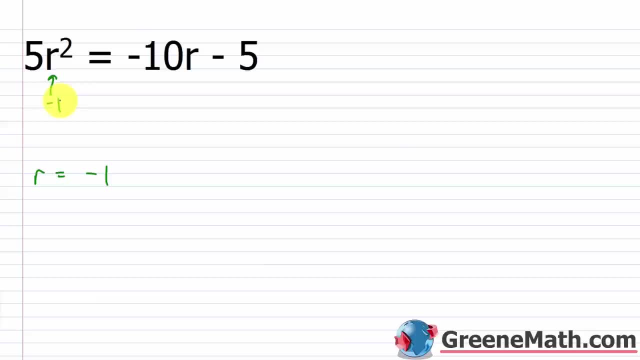 r is equal to negative 1, so if I plug that in here and here, I'd have 5 times negative 1 squared is equal to negative 10 times negative 1 minus 5. Negative 1 squared is 1, 5 times 1 is 5, and this equals negative 10 times negative 1 is 10, and then minus 5, 10 minus 5 is 5, so you get 5 equals 5, so this solution checks out. r is equal to negative 1. 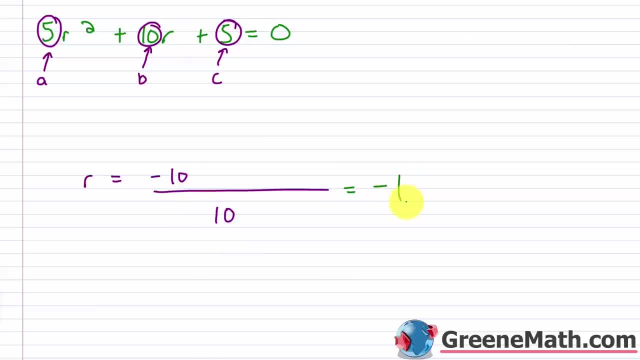 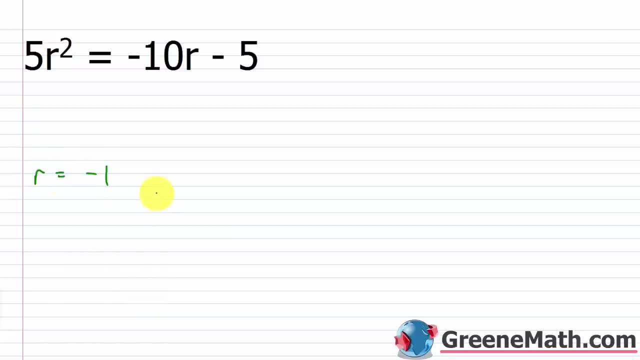 So here r is equal to negative 10 over 10, which is negative 1.. And that's a simple one to check, So let's go ahead and do that. So again, r is equal to negative 1.. So if I plug that in here and here, I'd have 5 times negative. 1 squared is equal to negative 10 times negative 1 minus 5.. 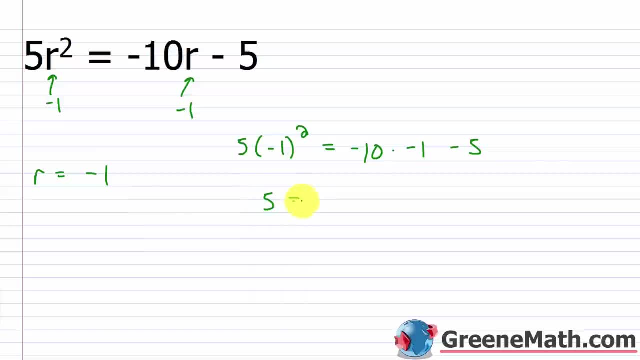 Negative 1 squared is 1.. 5 times 1 is 5. And this equals negative. 10 times negative, 1 is 10.. And then minus 5.. 10 minus 5 is 5.. So you get 5 equals 5.. 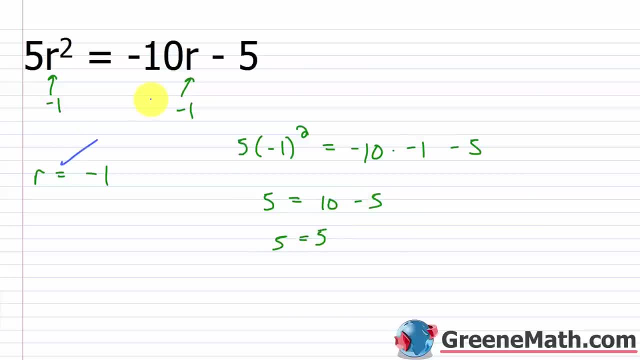 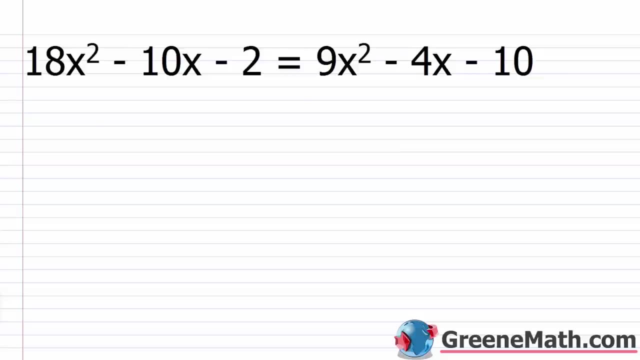 So this solution, This solution checks out: r is equal to negative 1.. All right, Let's take a look at another one. So we have: 18x squared minus 10x minus 2 is equal to 9x squared minus 4x minus 10.. 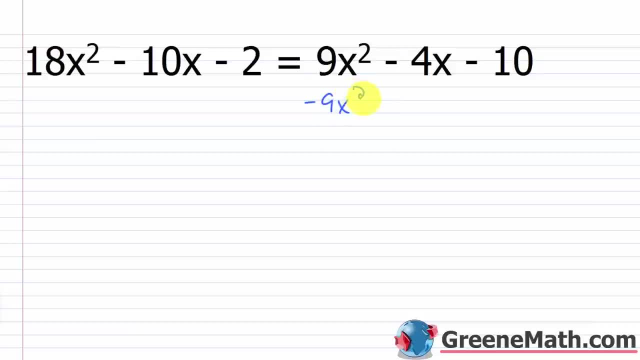 Really, all I have to do is subtract 9x squared away from each side of the equation. That'll cancel. Add 4x to each side of the equation- That'll cancel. And add 10 to each side of the equation. 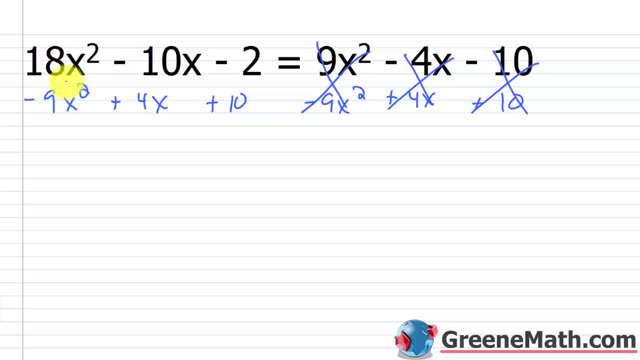 That'll cancel over there. So I'd have 18x squared minus 9x. 9x squared is 9x squared Negative. 10x plus 4x is negative, 6x Negative. 2 plus 10 is positive 8.. 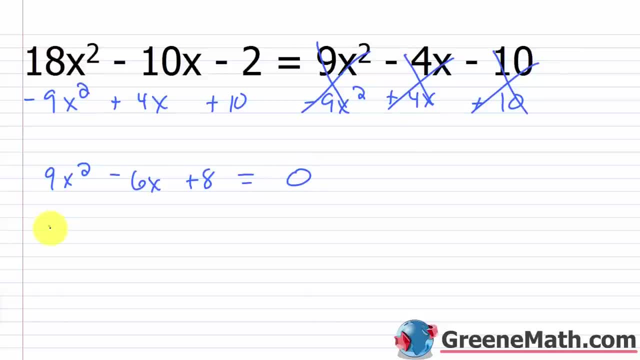 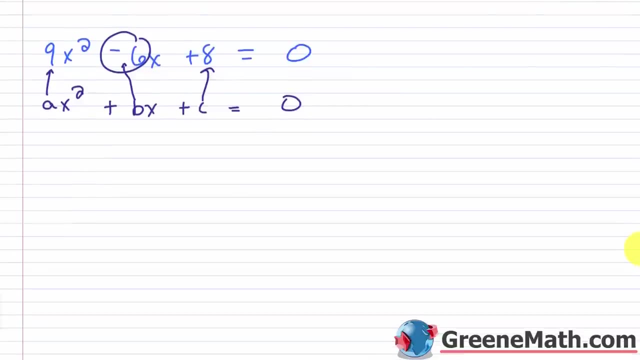 And this equals 0.. And so this is, in standard form, right. We have ax squared plus bx plus c equals 0.. We have a is 9.. b is negative 6. And c is 8.. So if I plug into my quadratic formula, what am I going to get? 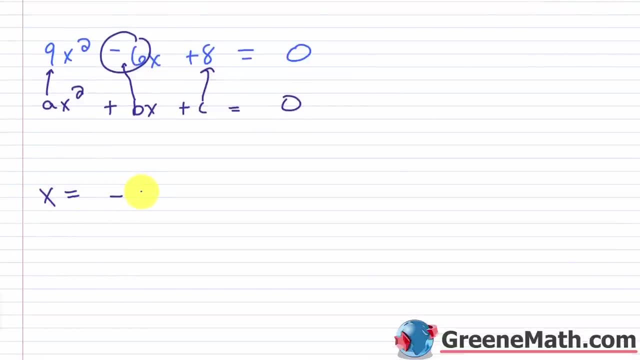 I get that x is equal to Negative b, So in this case b is negative 6.. So the negative of negative 6 is plus 6.. Plus or minus the square root of b squared. If I square negative 6, I get 36.. 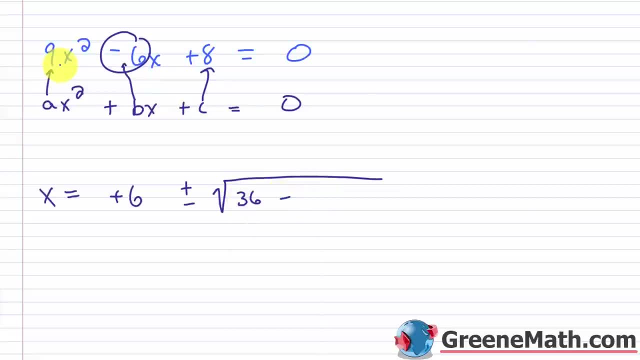 Minus 4 times a, a is 9.. 4 times 9 is 36.. Times c: c is 8.. So 36 times 8 is 288.. Now you already can see you're going to have a problem. 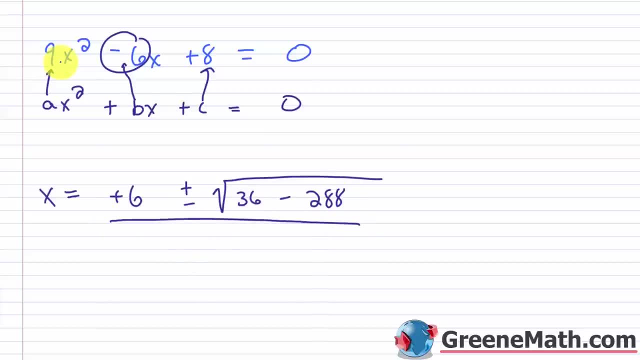 But let's continue. This is over 2 times a. a is 9.. So 2 times 9. is 18.. Now why did I say that you're going to have a problem If 36 minus 288 is a negative value and it's negative 252,? 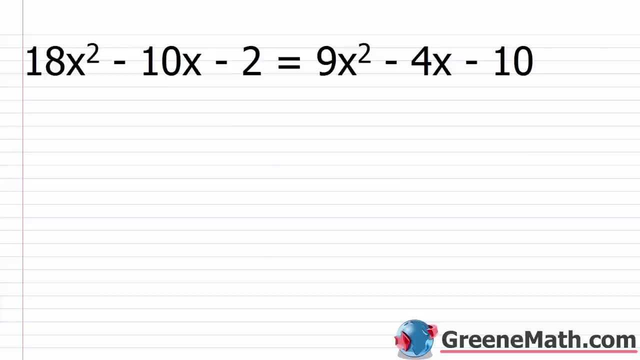 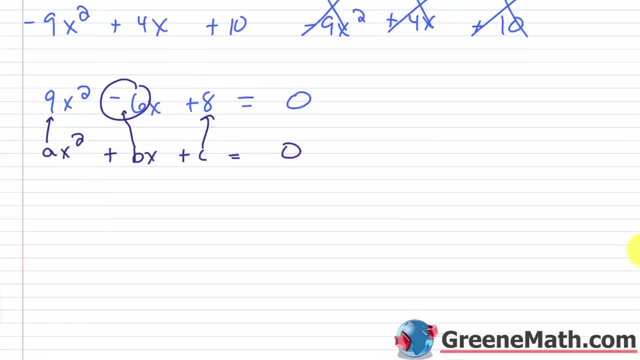 All right, let's take a look at another one. So we have 18x squared minus 10x minus 2 is equal to 9x squared minus 4x minus 10. Really, all I have to do is subtract 9x squared away from each side of the equation. That'll cancel. Add 4x to each side of the equation. That'll cancel. And add 10 to each side of the equation. That'll cancel over there. So I'd have 18x squared minus 9x squared is 9x squared. Negative 10x plus 4x is negative 6x. Negative 2 plus 10 is positive 8 and this equals 0, and so this is in standard form. We have ax squared plus bx plus c equals 0. We have a is 9 b is negative 6 and c is 8. So if I plug into my quadratic formula, what am I gonna get? I get that x is equal to negative b. 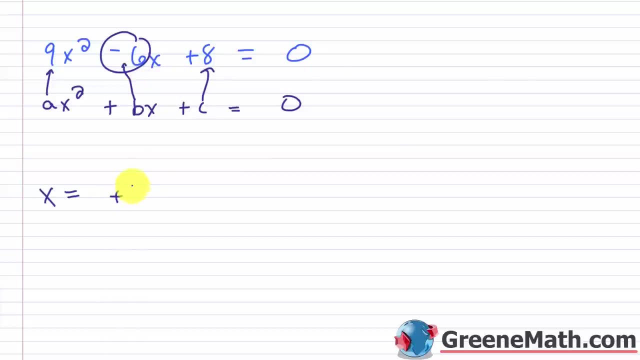 So in this case b is negative 6, so the negative of negative 6 is plus. 6 plus or minus the square root of b squared by squared negative 6 I get 36 minus 4 times a a is 9 4 times 9 is 36 times C C is 8 so 36 times 8 is 288 now 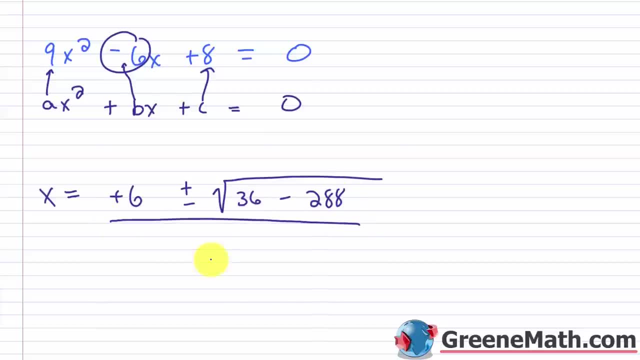 you already can see you're gonna have a problem but let's continue this is over 2 times a a is 9 so 2 times 9 is 18 now why did I say that you're gonna have a 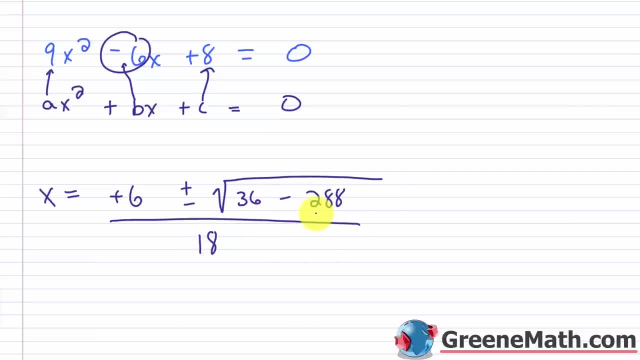 problem if 36 minus 288 is a negative value and it's negative 252 can I take the square root of a negative number well I can but not yet the solution is not a real number in this particular case we'd stop and say there's no real 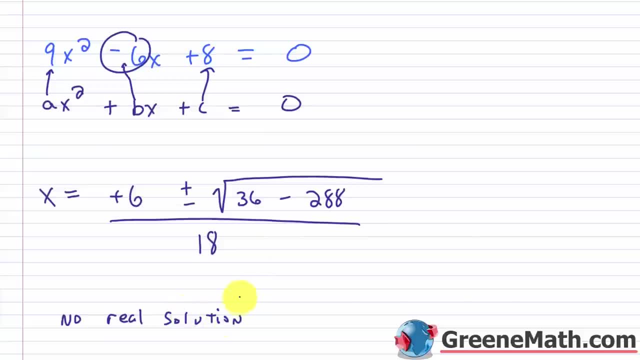 solution okay so this is gonna come up pretty often until you start dealing with complex numbers and then you actually will be able to get a solution but we haven't gotten to that yet so for right now we just need to figure out how to solve this problem and then we'll get to the solution but we haven't gotten to that yet so for right now we just need to 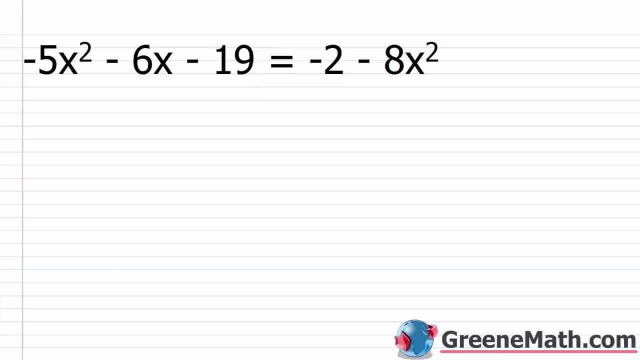 stop and say there's no real solution all right let's take a look at no so we have negative 5x squared minus 6x minus 19 equals negative 2 minus 8x squared so 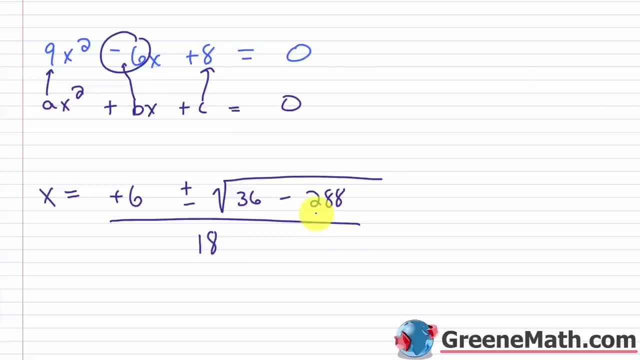 can I take the square root of a negative number? Well, I can, but not yet. The solution is not a real number. In this particular case, we'd stop and say there's no real solution. So this is going to come up pretty often until you start dealing with complex numbers. 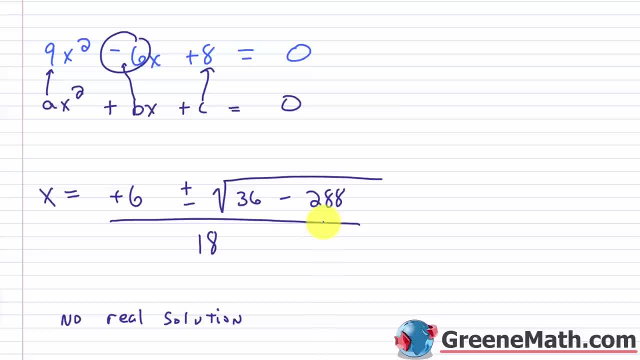 And then you actually will be able to get a solution. But But we haven't gotten to that yet. So for right now we just stop and say there's no real solution. All right, Let's take a look at another one. 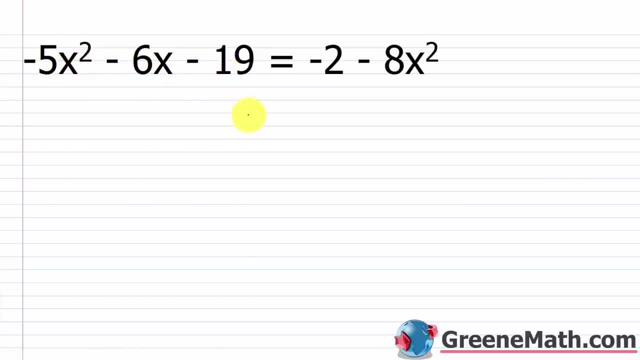 So we have negative 5x squared minus 6x minus 19 equals negative 2 minus 8x squared. So I'm going to add 8x squared to each side of the equation. That'll cancel. I'm going to add 2 to each side of the equation. 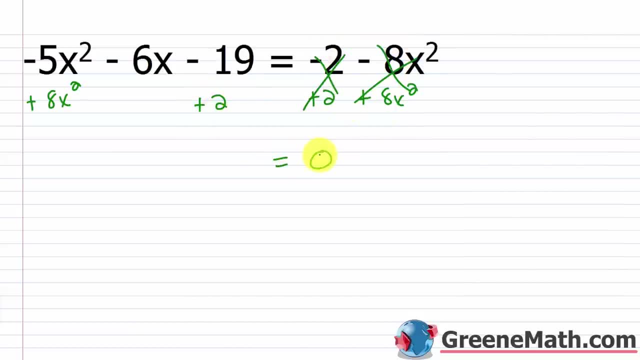 That'll cancel. So I'll have 0 on the right. On the left: 8x squared minus 5x squared is 3x squared. Minus 6x squared is 3x squared. Minus 6x squared is 3x squared. 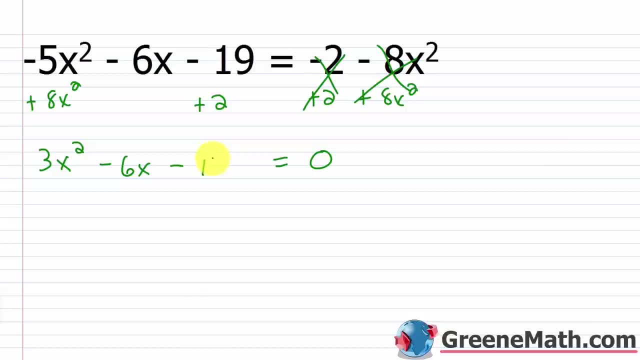 Minus 6x and then negative. 19 plus 2 is negative 17.. At this point you should be kind of getting this. This is ax squared plus bx plus c equals 0.. A is the coefficient for the squared variable. 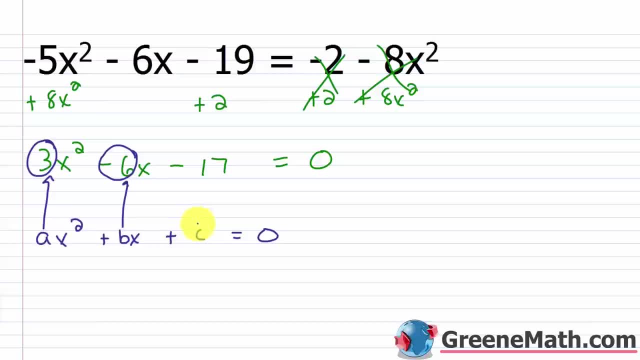 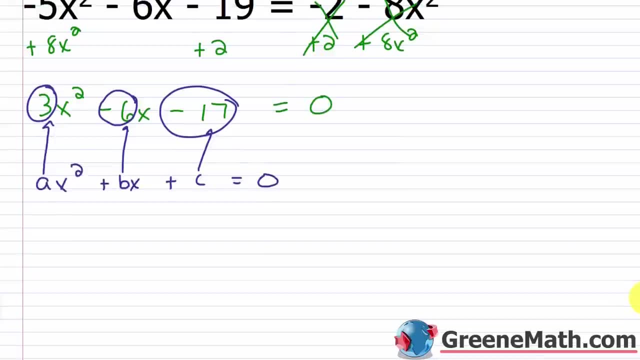 B is the coefficient for the variable to the first power, And then c is the constant. OK, Make sure you include the negatives, Otherwise you won't get the right answer. All right, So the quadratic formula, Remember. So x is equal to the negative of b. 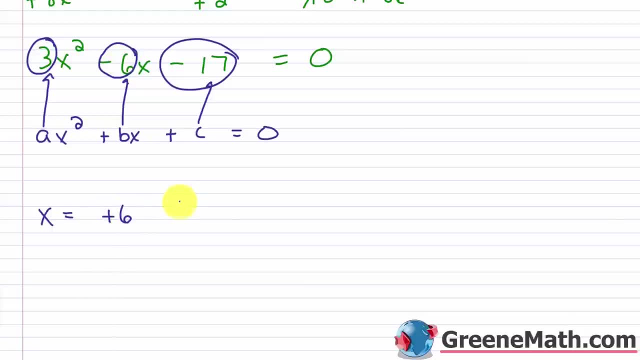 b is negative 6.. So the negative of negative 6 is plus 6.. Plus or minus the square root of b squared By square b, I get 36.. Minus 4 times a, a is 3.. 4 times 3 is 12.. 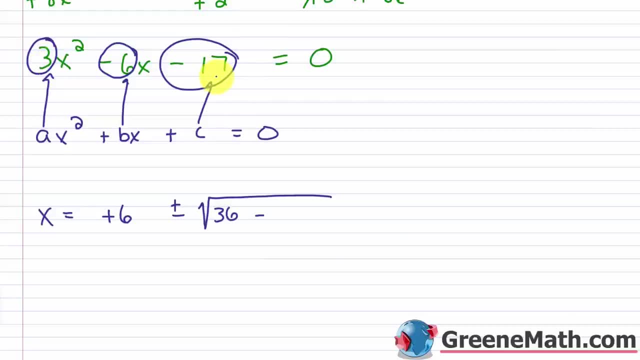 Times c, 12 times negative, 17 is negative 204.. So minus the negative 204 is plus 204.. OK, So I would get 36 plus 204, which is 240.. So this is plus or minus the square root of 240.. 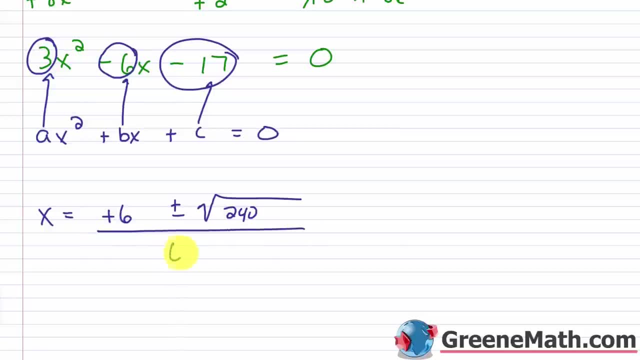 And this is over 2 times a. a is 3.. So 2 times 3 would be 6.. All right, So now, what is the square root of 240?? Well, 240 is not a perfect square. 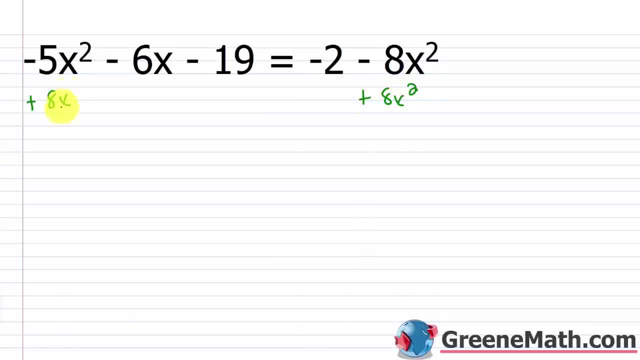 I'm gonna add 8x squared to each side of the equation that'll cancel I'm gonna add 2 to each side of the equation that'll cancel so I'll have 0 on the right on the left 8x squared minus 5x squared is 3x squared minus 6x and then negative 19 plus 2 is negative 6x squared minus 3x squared minus 3x squared is negative 17 at this point you should be kind of getting this this is ax squared plus B X plus C equals 0 a is the coefficient for the squared variable 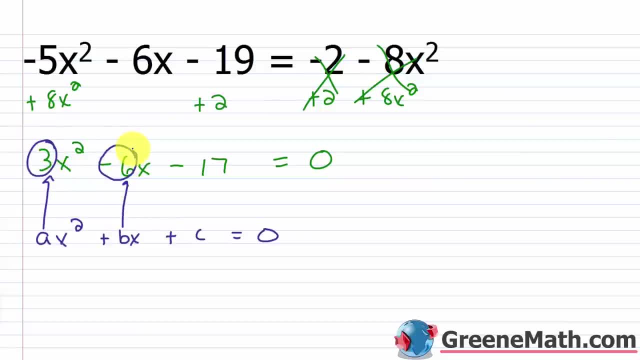 B is the coefficient for the variable to the first power and then C is the constant okay make sure you include the negatives otherwise you won't get the 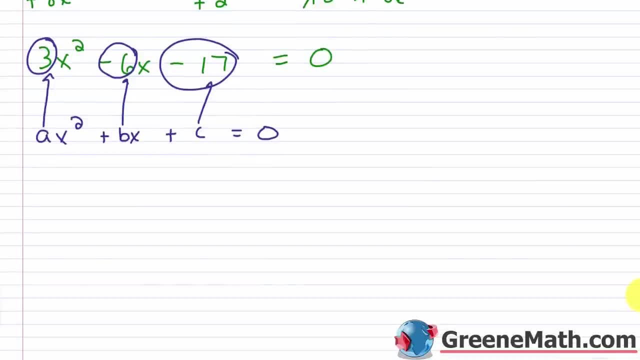 right answer alright so the quadratic formula remember it's X is equal to the negative of B B is negative 6 so the negative of negative 6 is plus 6 plus or minus the square root of B squared by square B I get 36 minus 4 times a a is 34 times 3 is 12 times C 12 times negative 17 is negative 204 so minus a negative 204 is plus 204 so I would get 36 plus 204 which is 240 so this is plus or minus the square root of 240 and this is over 2 times a a 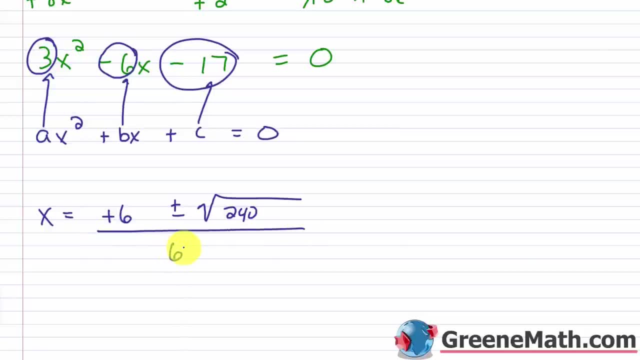 is 3 so 2 times 3 would be 6 all right so now what is the square root of 240 well 240 is not a perfect square so here we get something that's gonna be kind of messy so for 240 I'll factor that to 24 times 10 and let me factor this into 6 times 4 I know that's a little bit too much but I'm gonna do that so I'm gonna factor that to 24 times 10 and let me factor this into 6 times 4 I know that's a little bit too much but I'm gonna do that so I'm gonna do that so I'm gonna 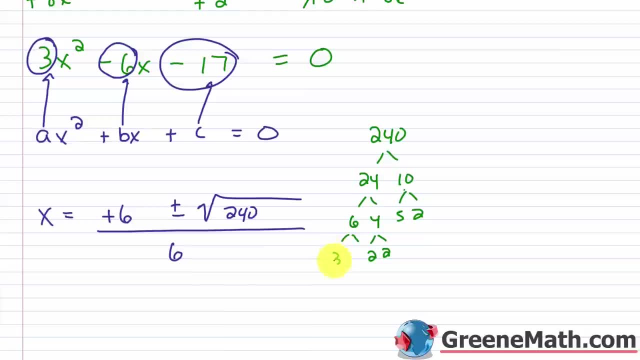 this is 5 times 2 this is 2 times 2 this is 3 times 2 so I have 1 2 3 4 this is 5 times 2 this is 2 times 2 this is 3 times 2 so I have 1 2 3 4 factors of 2 so I'm gonna have 16 times 15 16 times 15 so I know 16 is a 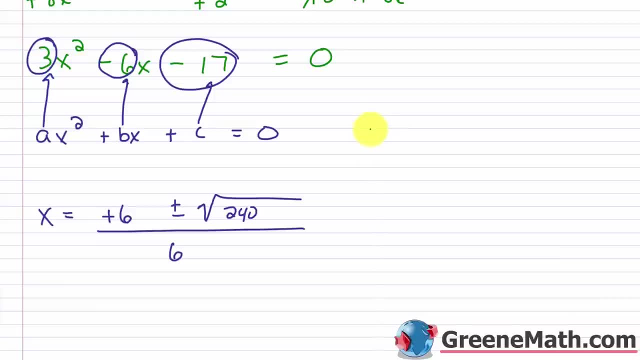 So here we get something that's going to be kind of messy. So for 240, I'll factor that to 24 times 10.. And let me factor this into 6 times 4.. I know this is 5 times 2.. 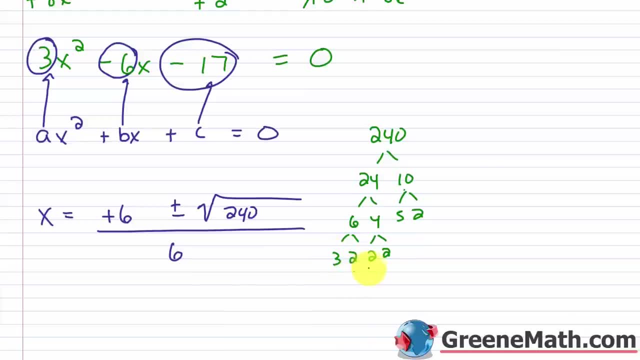 This is 2 times 2.. This is 3 times 2.. So I have 1,, 2,, 3,, 4 factors of 2.. So I'm going to have 16 times 15.. 16 times 15.. 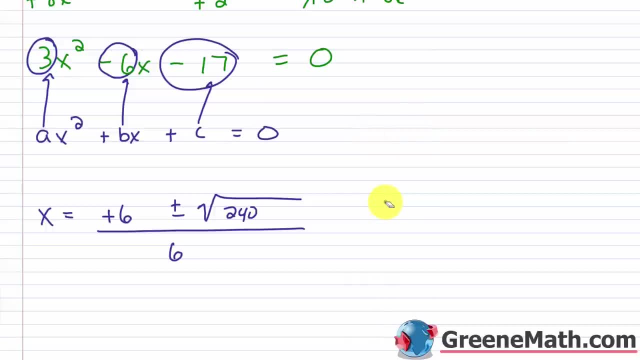 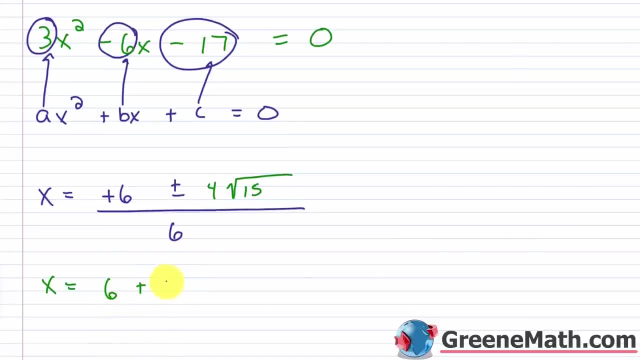 So I know 16 is a perfect square. Square root of 16 would be 4.. So basically I could write this as 4 times the square root of 15.. Now I just have two scenarios I will have. x is equal to 6 plus 4 times square root of 15 over 6.. 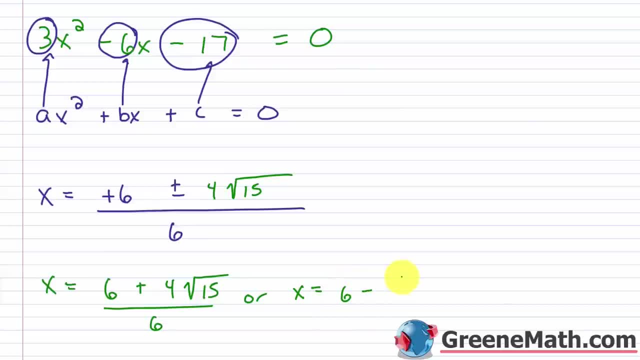 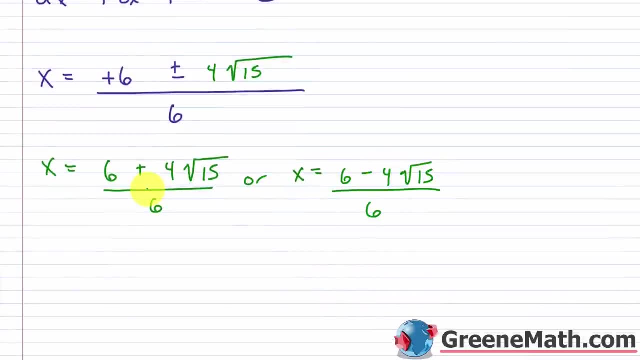 Then, or x equals 6 minus. OK, let me scroll down 4 times the square root of 15 over 6.. And we can further simplify these. What we can do is we can factor 2 from the numerator, So I can put 2 times 3 plus 2 times square root of 15.. 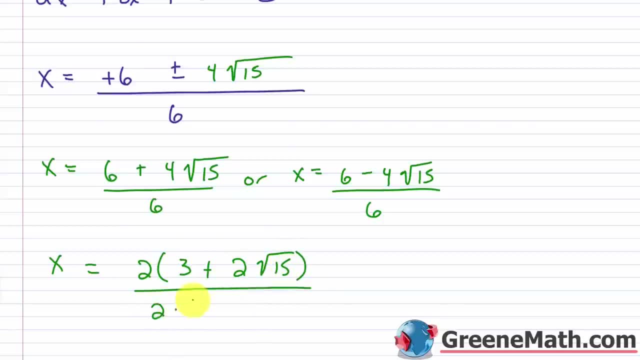 OK, 15 over 2 times 3.. So this would cancel with this and I'd be left with 3 plus 2 times square root of 15 over 3.. It'd be the same thing over here If I cancel out a common factor of 2,. this would be a 3,, this would be a 2, and this: 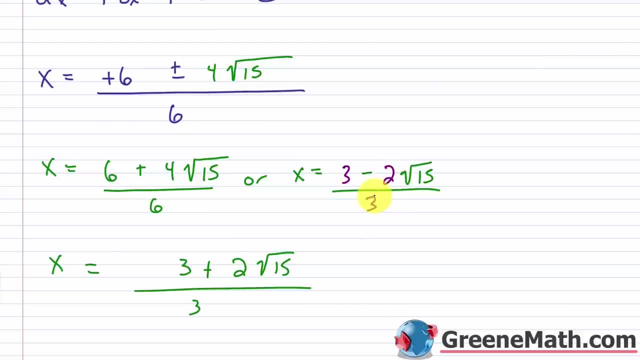 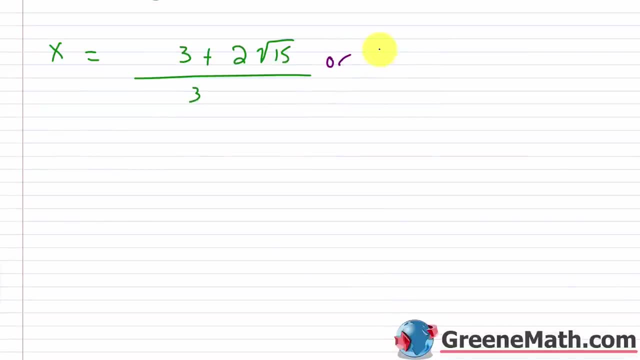 would be a 3 down here, So I can have x equals 3 plus 2 times square root of 15 over 3, or x equals 3 minus 2 times square root of 15 over 3.. Those would be your two solutions. 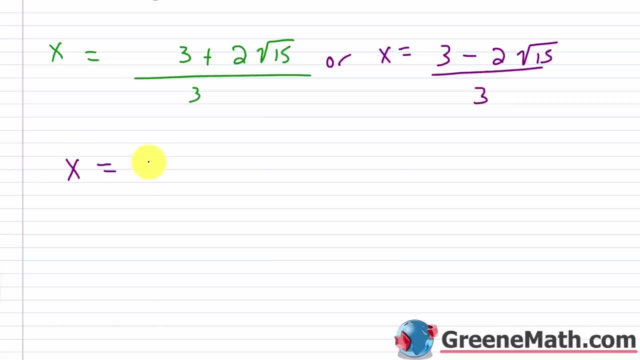 And of course you could write that in a more compact format by just saying: x equals 3 plus or minus 2 times square root of 15 over 3.. Now I could check this answer, but in the interest of time I'm not, because something 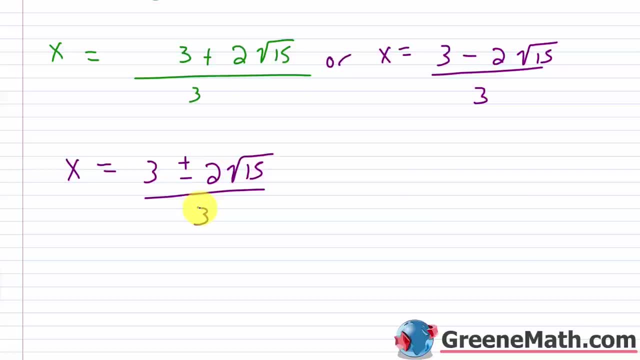 like that gets really confusing. It's really really tedious. If you want some practice- and I think it is good to practice with things like that- pause the video, take each one of these and plug it in for x in the original equation. 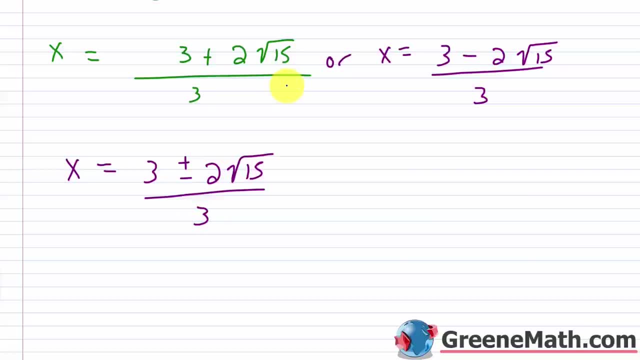 and see that you get the left and the right side as the same value. factors of 2 so I'm gonna have 16 times 15 16 times 15 so I know 16 is a 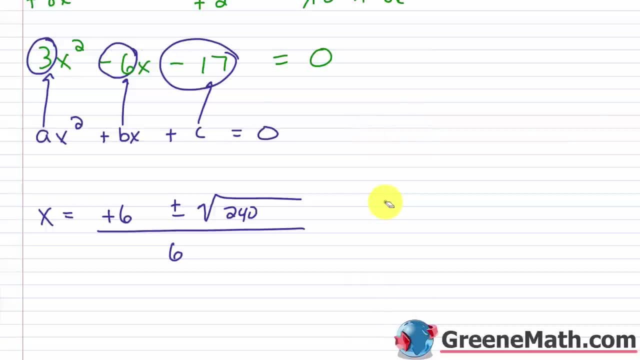 perfect square square root of 16 would be 4 so basically I could write this as perfect square square root of 16 would be 4 so basically I could write this as 4 times the square root of 15 now I just have two scenarios I will have X is 4 times the square root of 15 now I just have two scenarios I will have X is equal to equal to 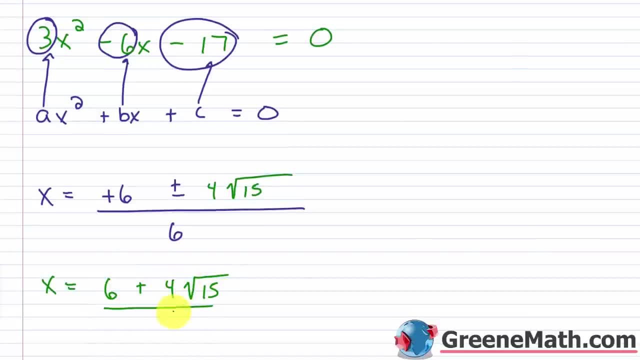 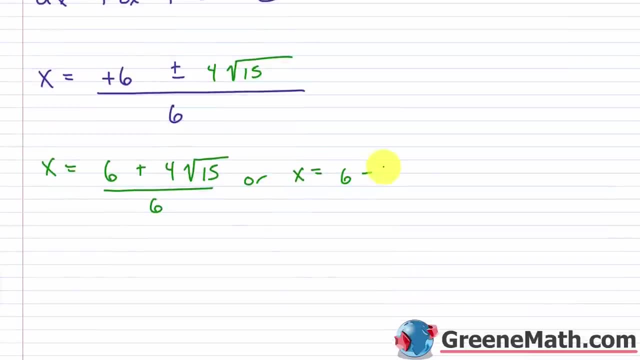 plus 4 times square root of 15 over 6 plus 4 times square root of 15 over 6 plus 4 times square root of 15 over 6 then or X equals 6 minus okay let me then or X equals 6 minus okay let me then or X equals 6 minus okay let me scroll down 4 times the square root of scroll down 4 times the square root of scroll down 4 times the square root of 15 over 6 and we can further simplify 15 over 6 and we can further simplify 15 over 6 and we can further simplify these what we can do is we can factor 2 these what we can do is we can factor 2 these what we can do is we can factor 2 from the numerator so I can put 2 times from the numerator so I can put 2 times from the numerator so I can put 2 times 3 plus 2 times square root of 15 over 2 3 plus 2 times square root of 15 over 2 3 plus 2 times square root of 15 over 2 times 3 so this would cancel with this 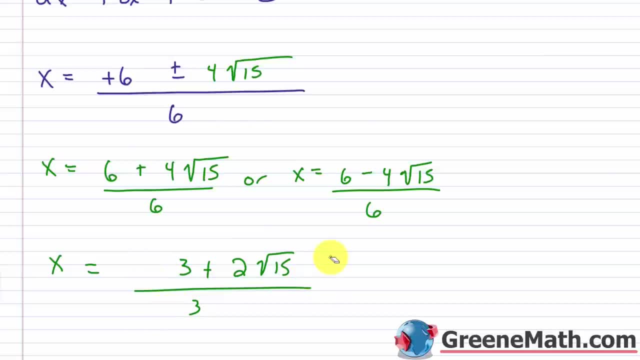 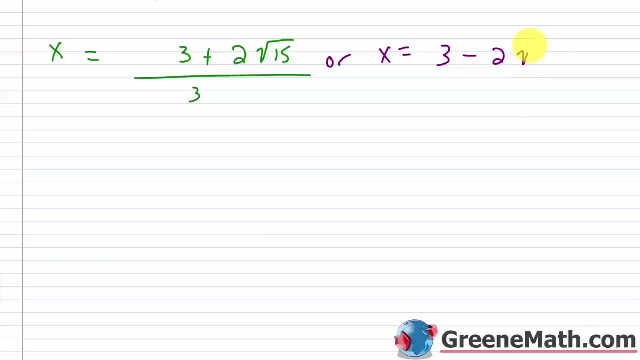 2 times square root of 15 over 3 or X equals 3 minus 2 times square root of 15 equals 3 minus 2 times square root of 15 equals 3 minus 2 times square root of 15 over 30 those would be your two over 30 those would be your two over 30 those would be your two solutions and of course you could write solutions and of course you could write solutions and of course you could write that in a more compact format by just that in a more compact format by just that in a more compact format by just saying X equals 3 plus or minus 2 times saying X equals 3 plus or minus 2 times saying X equals 3 plus or minus 2 times square root of 15 over 3 now I could square root of 15 over 3 now I could square root of 15 over 3 now I could check this answer but in the interest of check this answer but in the interest of check this answer but in the interest of time I'm not because something like that